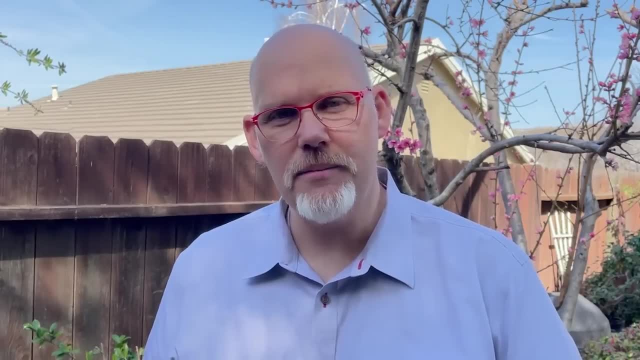 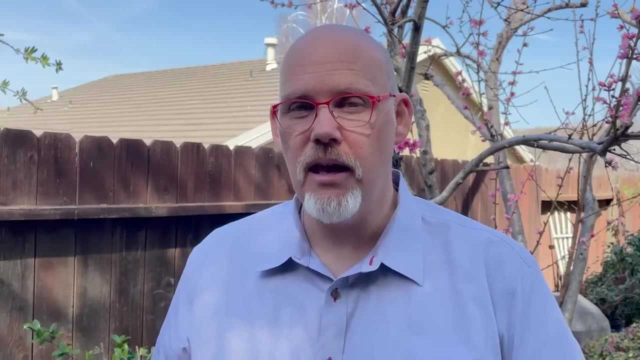 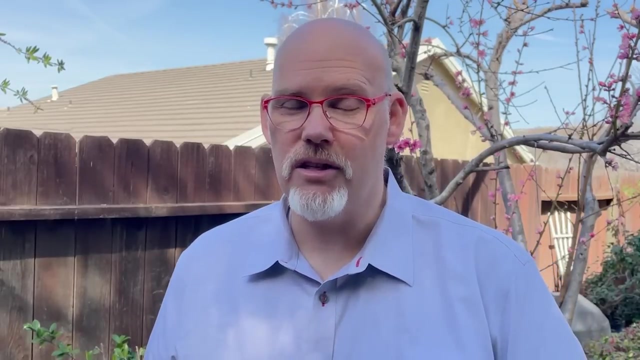 And that's really interesting to see how a language has evolved and developed and how that affects the way you write modern, up-to-date JavaScript, And I think you'll learn a lot from this and you'll be able to do some interesting things with JavaScript as you go along, So stick. 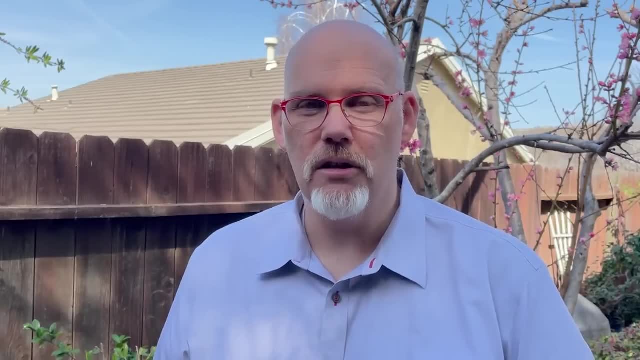 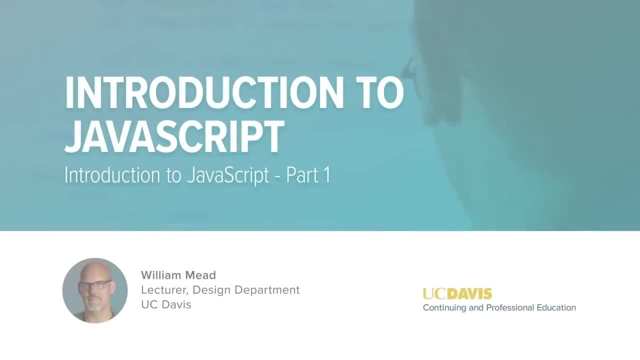 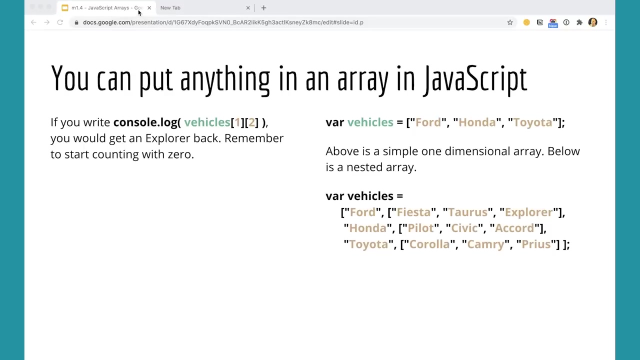 with me and we will have a lot of fun in this first module, learning about JavaScript and the basics of the language. Unlike a pillbox, which really can't hold much more than just pills, you can put anything into an array. in JavaScript, You can even put an array in an array. 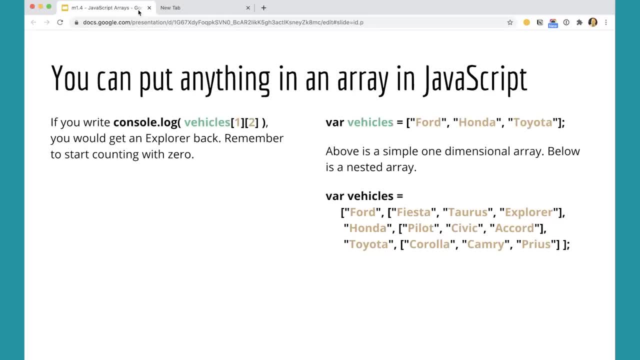 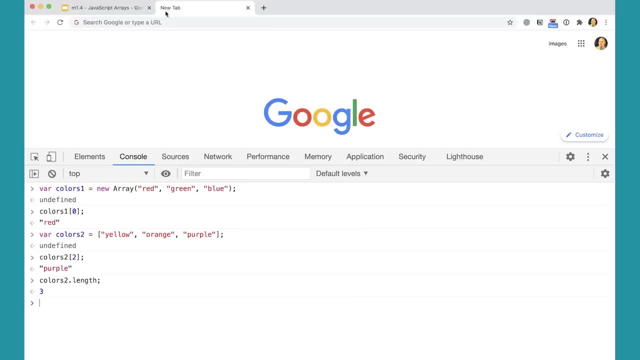 So you can think about a pillbox with a sub-container with even smaller divisions in it. So let's take a look at what that looks like. I'm going to switch back over to my tab here. I'm going to clear out this tab. 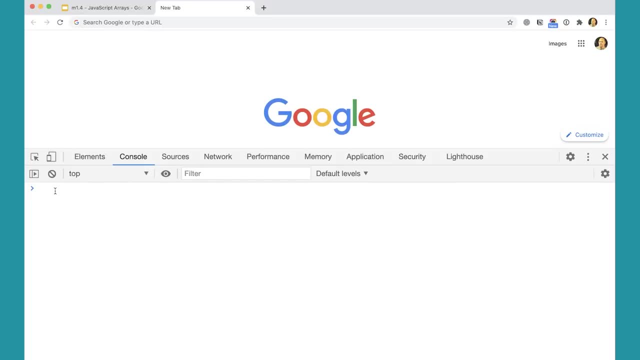 by clicking the Clear button there. I'm just going to paste this in, but you might want to type it. It's a little bit hard to type and get right, but it's worth trying. if you can, I'm going to paste this vehicles array in here. 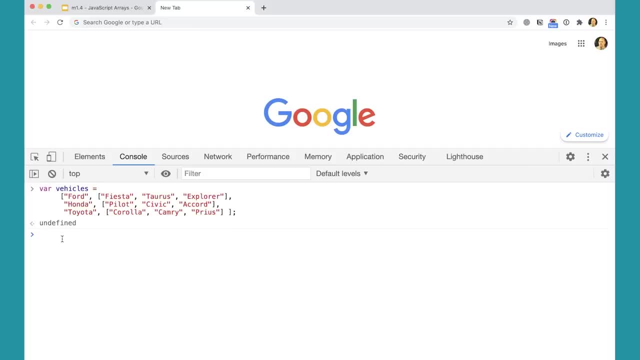 Now, if I want to access an element from this array, I could do vehicles, square, bracket one. That's going to go and get the line that starts with which element. There we go. It's going to get me this, because this is zero and now this is one. 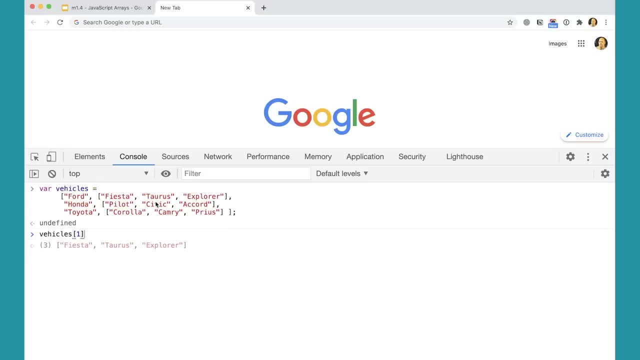 That's going to get me into that subarray. You can see it's showing up down there. Then if I do square bracket two, that's going to get me the explorer element in that subarray, So you can do things like that with arrays. 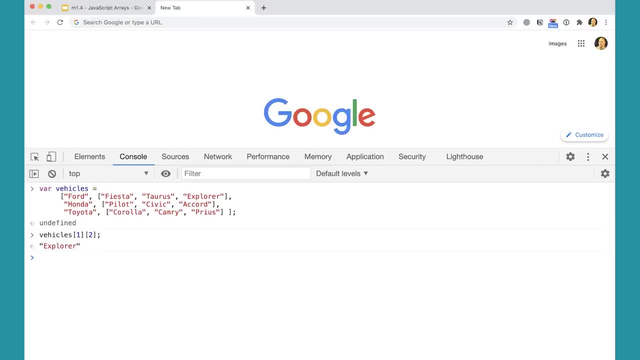 That's complicated and you're not probably going to be doing arrays inside of arrays to start off with, but it's an important thing to understand about arrays. They're very flexible tools that you can use to hold groups of data and that's very useful. 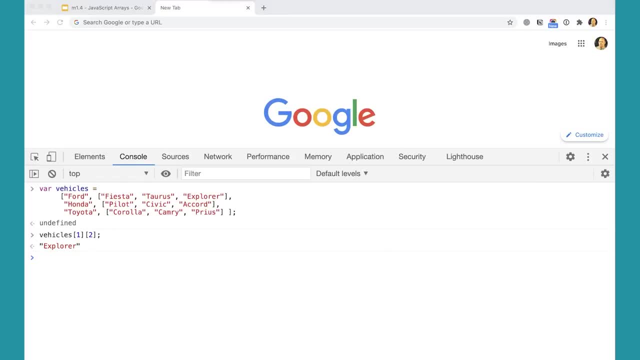 Another thing that's interesting is that a regular variable holding a string can be treated like an array in JavaScript. So if I make a variable, var joke equals the chicken crossed the road. the chicken crossed the road. I can save my string. Let's make a variable. 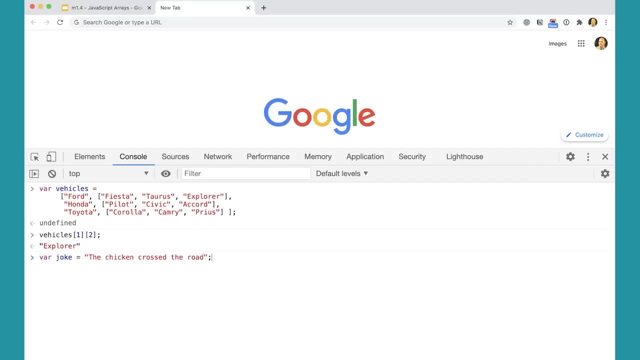 The chicken crossed the road So I can save my string. I can save my string. It's pretty easy. I can save my string. Now I've got a variable called joke, but I can actually treat it like an array. I could do joke square, bracket four, and that's going to get me the C in chicken, because 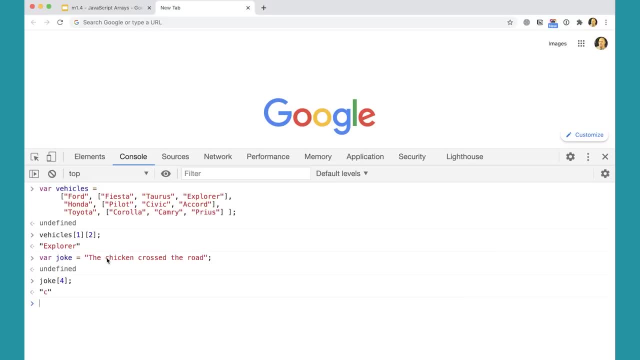 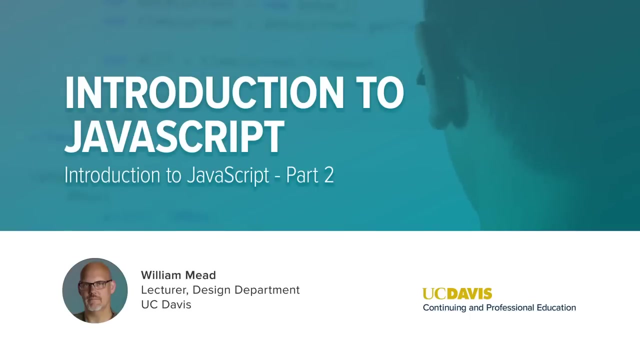 zero one, two, three, four is going to get me that C in chicken, Or I could do joke dot length and it'll tell me that there are 28 characters in that string. So that's kind of an interesting thing to understand about arrays as well. 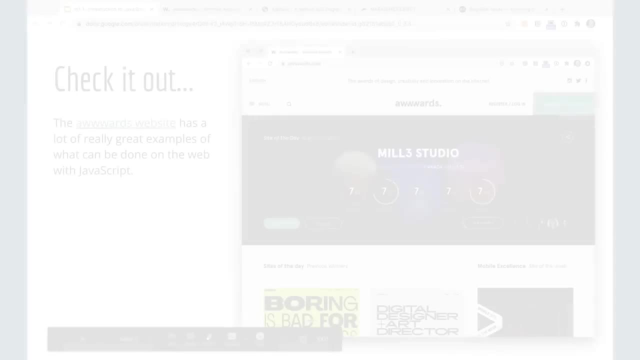 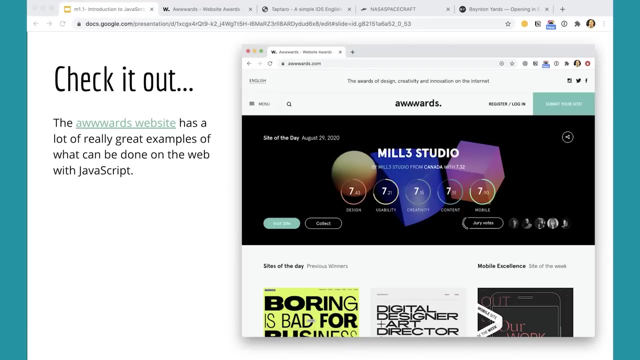 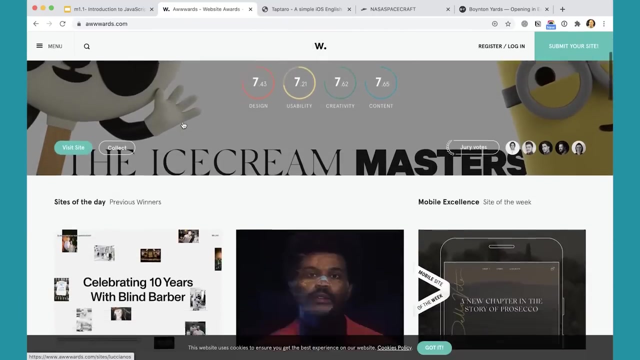 A great place to go to find some websites that will show you the way JavaScript can interact with a website is this awards website. It's a website with the extra Ws in here and I have that website pulled up over here And you can come here and look through some of the different sites that have won awards. 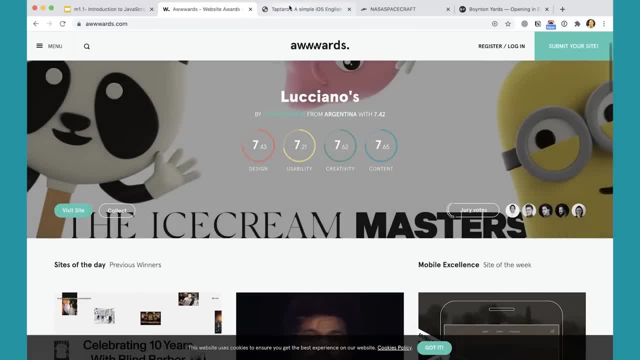 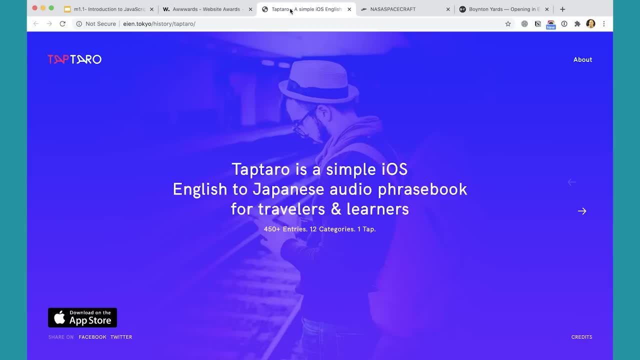 and they tend to be pretty innovative and interesting sites. I have a few that I just pulled up just now. These aren't pulled up for any special reason, other than that I looked at them and I thought that they had some interesting interactions, whether you're talking about following a mouse. 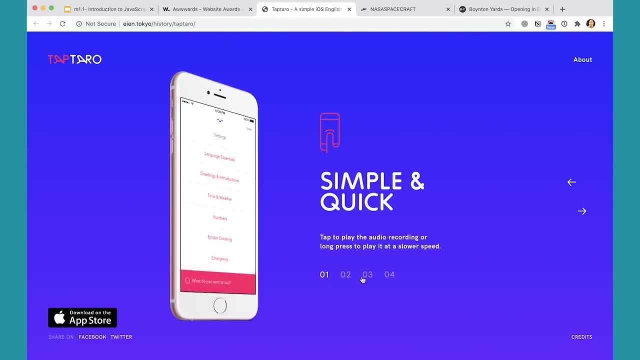 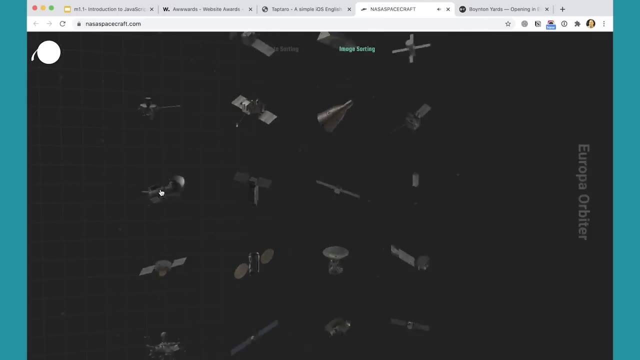 or coming over here and the animation around the circle, Or the way these images pop in. This is all being done with JavaScript, this kind of thing. And then here we are on one of the NASA spacecraft websites here and click on one of these things. 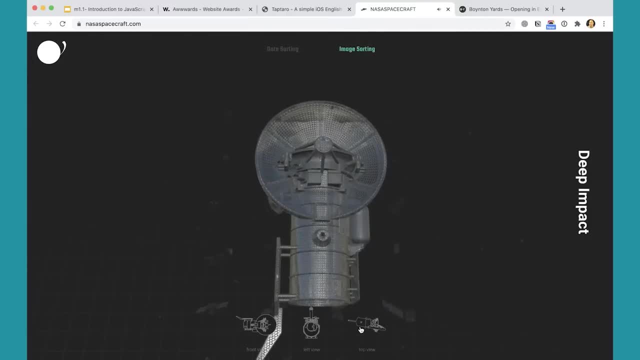 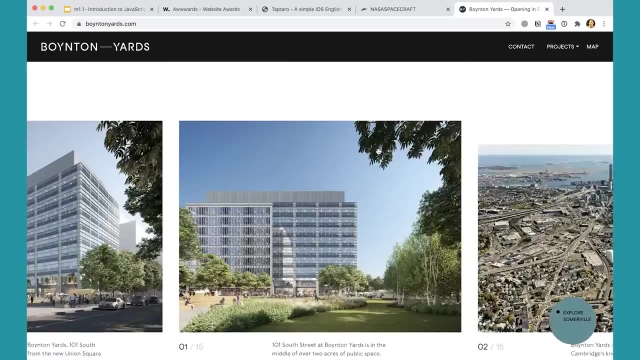 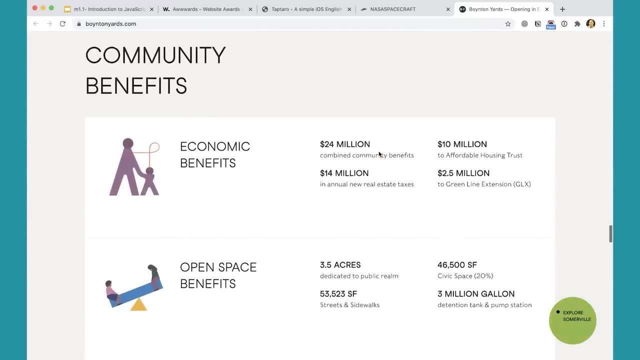 and it'll come up and show you the different pictures and give you some other interactions, including some sounds as you work around it. Or this website over here which, as you scroll through, does some interesting interactions As you're scrolling through the website. that kind of stuff. 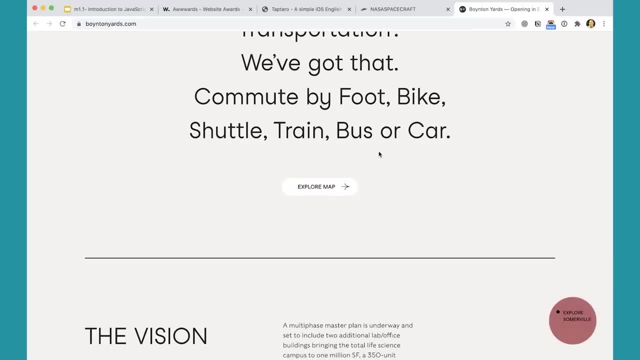 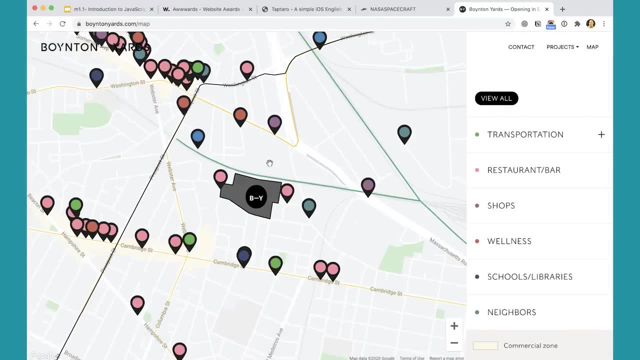 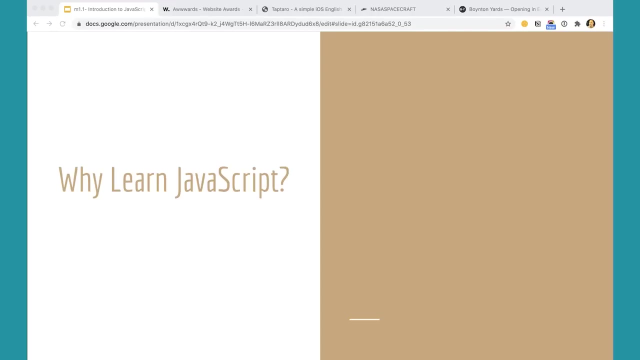 So, yeah, look around on the web and wherever you see interactions happening- whether it's a map like this or all kinds of interactions are being created by JavaScript. Great, You've seen some interactions in websites and you've probably seen plenty of others in other websites or gone off and found your own. 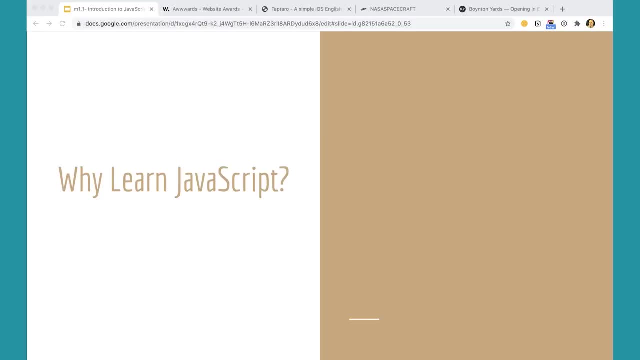 But let's talk about some other reasons why we should learn JavaScript. First of all, it's the most popular programming language in the world, and that's a really exciting thing to find out about JavaScript and a good reason to learn JavaScript. There's also a low barrier of entry to the field, whereas if you're learning Java or 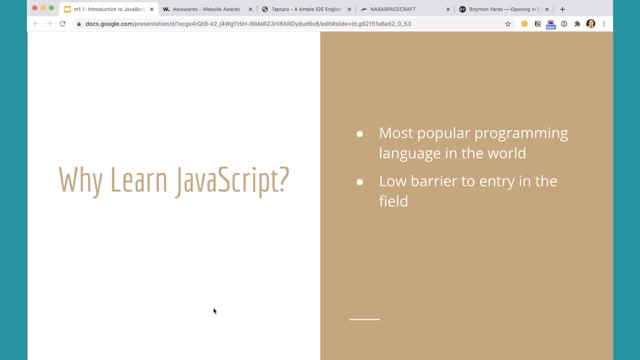 C or C++, you're going to need a lot of information, A lot of experience before you can get to a really good paying job. But JavaScript and the web is kind of the gateway to programming and to the tech industry in this way, So it's really good to learn JavaScript for that reason. 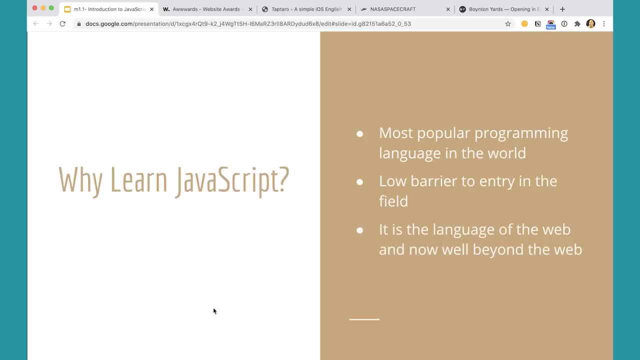 And then, finally, it is the language of the web. And now it goes well beyond the web. We have Raspberry Pi and other devices. They can all be programmed with JavaScript, robots and all kinds of things where JavaScript exists. Gaming engines: the Unity gaming engine uses JavaScript as well as C sharp. 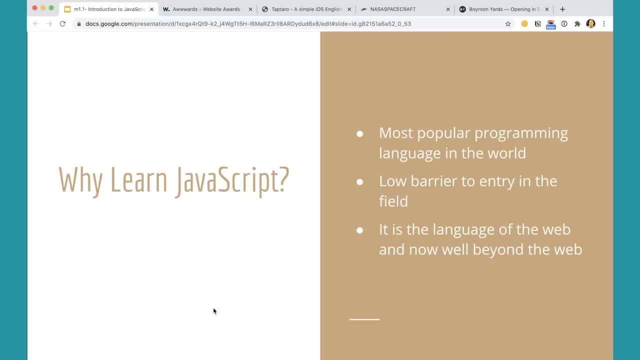 So there are lots of places where you can use JavaScript, but it is ultimately the language of the web. It is the programming, the scripting language for the web browser and it's native to the web browser. So that's a really great place to start. 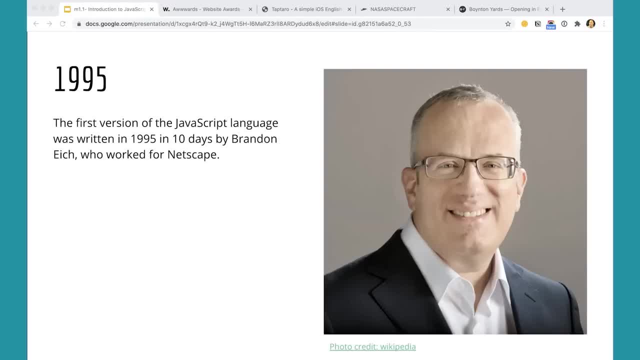 The story of JavaScript is really interesting. It really is the story of an underdog who became king. JavaScript didn't start off as the most popular programming language, And it's really important to understand this path that JavaScript has taken through history, because it has a big impact on how we write JavaScript. 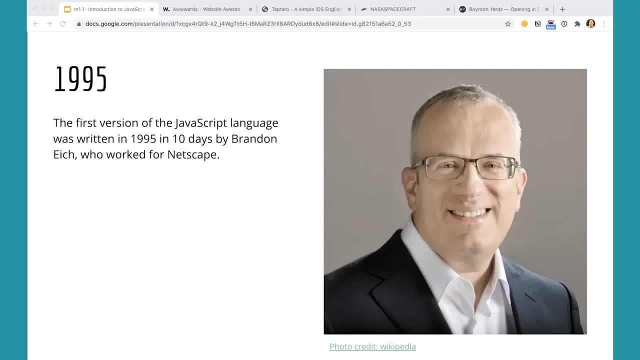 JavaScript was written by this man, This gentleman here, Brandon Eich, in 1995, over the course of ten days while he was working at Netscape, And I'm not going to go into great detail on the history here, but it's a really good. 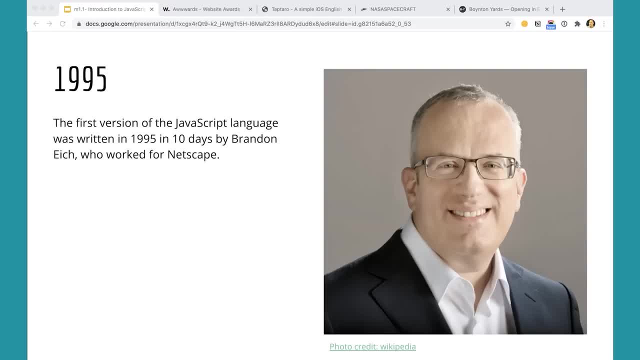 thing to look up. It's a very interesting story in and of itself, But he wrote the language in a very short amount of time and that's an important thing to understand about this language. Another important thing to understand about the JavaScript programming language: Is. it's not the same language as Java. It was originally a language called Mocha and they changed the name to JavaScript really as a marketing ploy, But it's not actually the same language as Java. They're two completely different languages. 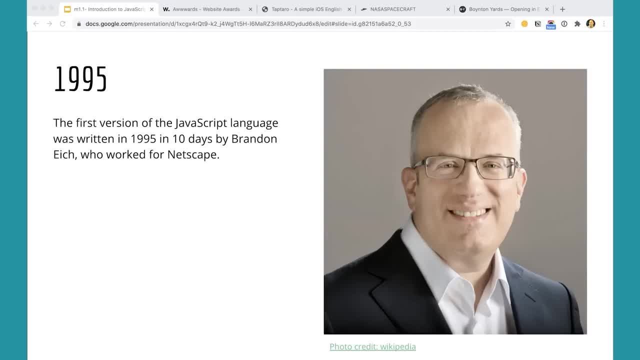 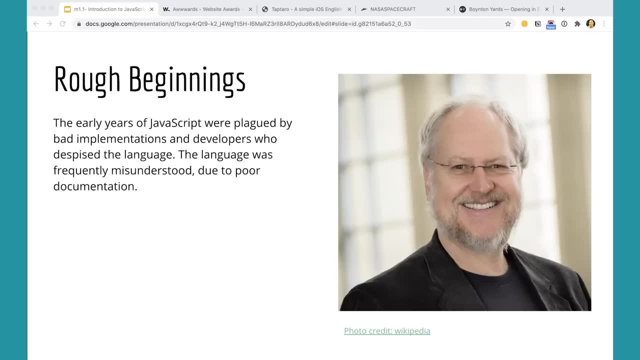 And it's easy as a beginner to get confused between Java and JavaScript. As I said before, JavaScript had some rough beginnings. The early years of JavaScript Were plagued by bad implementations, Developers who just despised the language, mostly due to poor documentation. 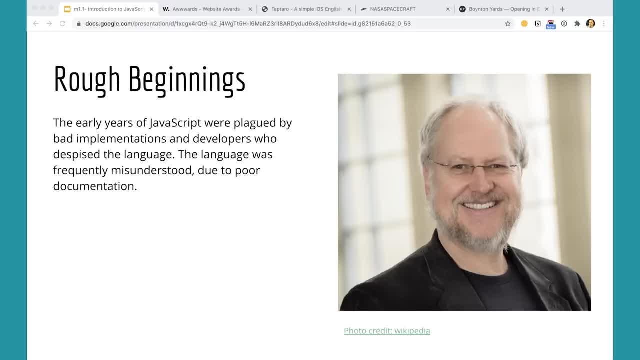 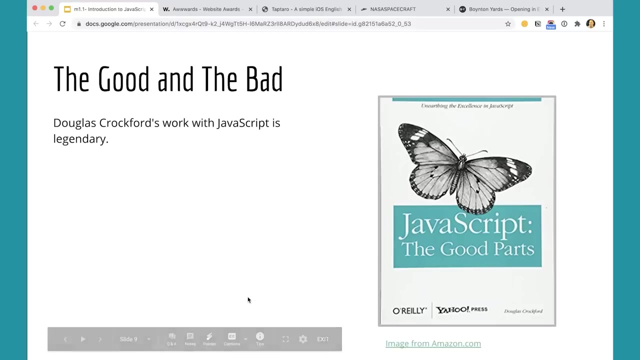 And it was greatly misunderstood as a language, And this gentleman, Douglas Crockford, did a lot to help people understand the incredible value of JavaScript as a language, and its strengths as well as its weaknesses. He wrote a book called JavaScript- The Good Parts, and it's a legendary book because 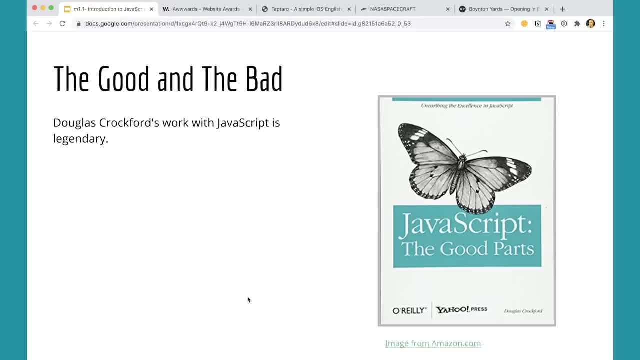 in this book he really talks about how JavaScript has some of the best features any programming language has ever had, Right alongside some of the worst features, and becoming a good JavaScript developer is about understanding how to leverage the best parts of the language while minimizing the. 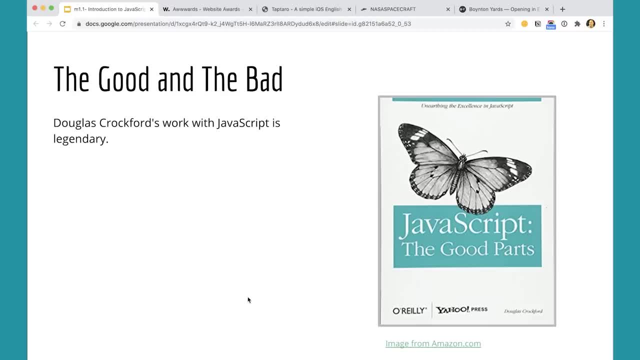 worst parts of the language And we'll be seeing some examples really quickly of some parts of the language that are good and not so good right off the bat And I'll be pointing those out And you'll see that as we go along we write JavaScript in ways to minimize the bad features. 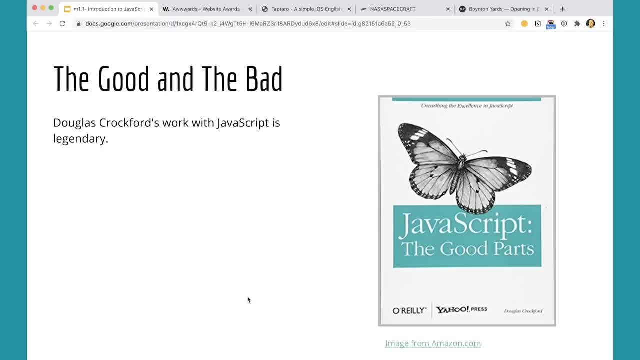 of the language, And when I say bad features, What I mean, I mean are features that can lead to more errors, lead to confusion in the programming, and so on and so forth. But it's also a very expressive language. It's a very powerful language. 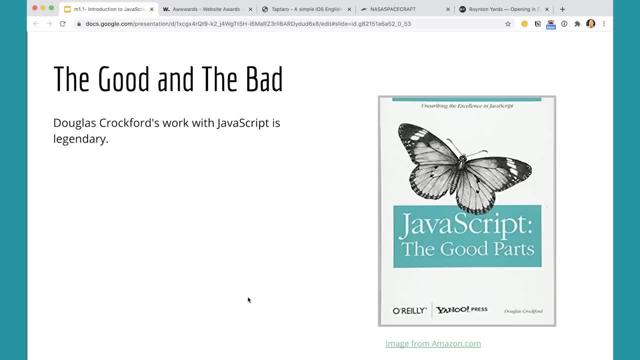 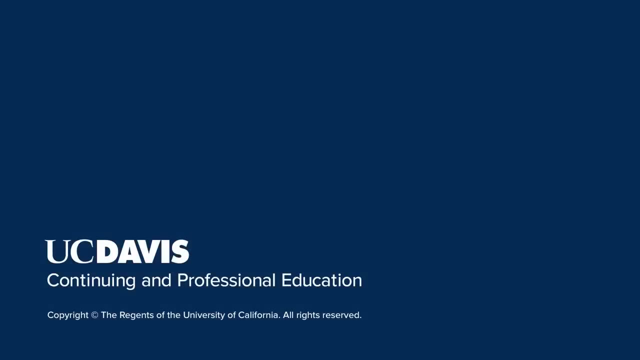 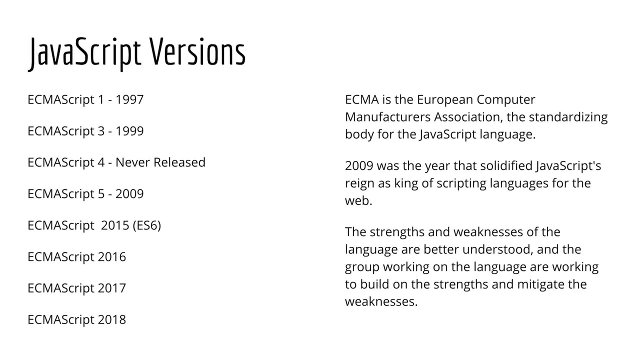 Some of the ideas behind it are very interesting and very powerful, even though they're different from other languages, which was behind some of the frustration that people had with it initially. They just didn't understand it because it was different. It's really important to understand the development of JavaScript over the years, and this is 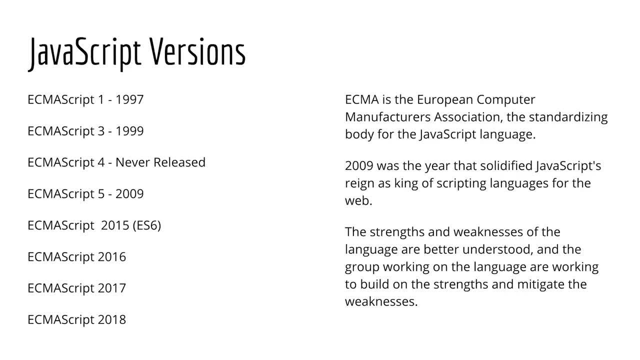 because the way JavaScript is developed has really impacted the way that we write JavaScript. So having a little bit of understanding of this history is really important as you learn the language. And again I'm just going to cover just the very basics, but there's a lot to this history. 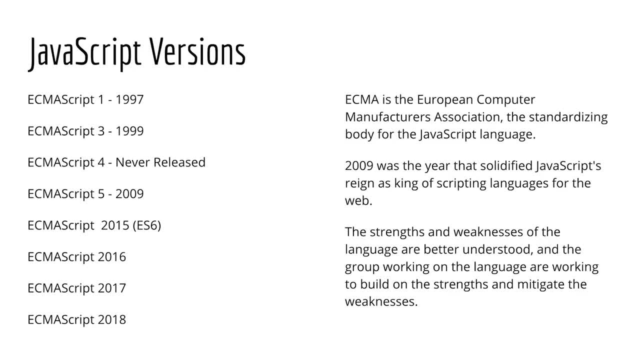 And it's a fascinating history and worth looking into if you're interested in that kind of thing, And you can find out about it by looking it up on the web or there's plenty of books about it and that kind of stuff. But just to be brief about it again, we know that JavaScript was originally written in. 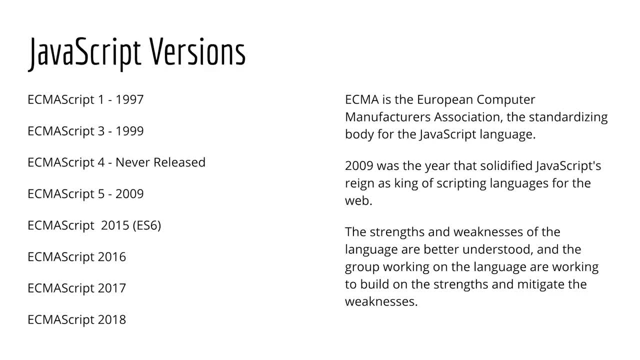 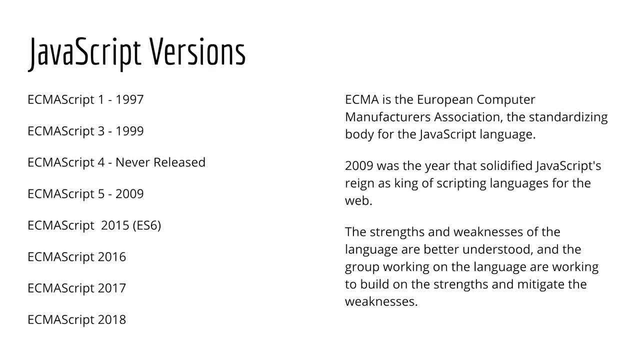 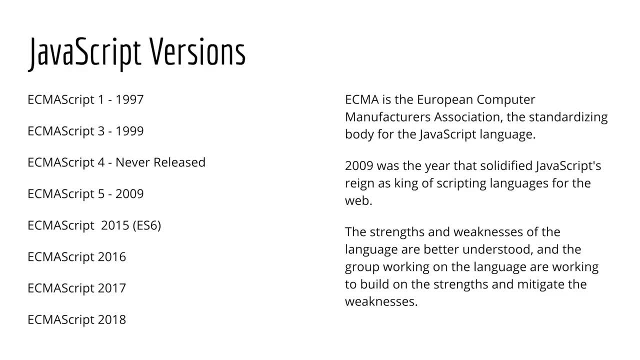 this language rubber stamped. It didn't turn out to be quite that easy, but that's a longer story. But in 1997, the first version, ECMAScript 1, was standardized and released And then a third version. the second version never really quite came out. 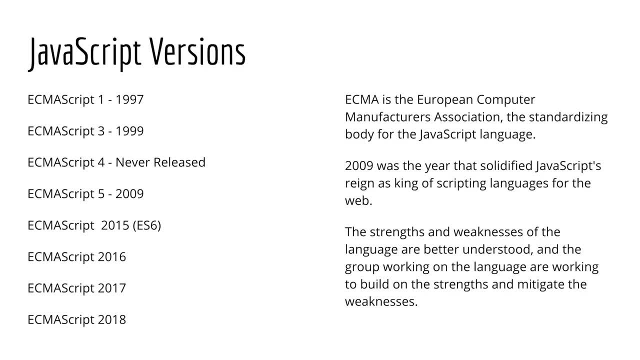 But in 1997, the first version, ECMAScript 1, was standardized and released. never really quite happened, but the third version came out in 1999 with some minor changes and fixes. The fourth version is an interesting story and one that I won't go into great depth. 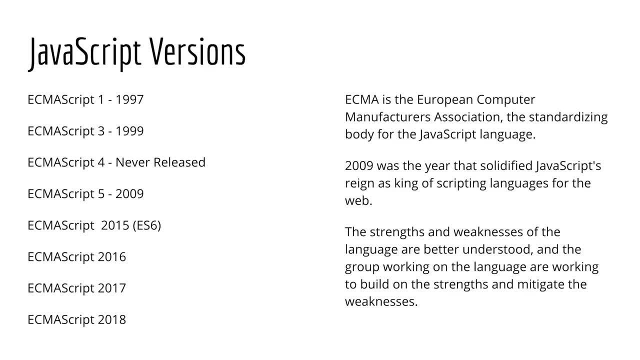 on, But again, you can look it up for yourself. But essentially, if you'll recall, I had said earlier that there was a lot of arguing about the direction of JavaScript and there were a lot of developers that didn't really understand it And there was some push to make JavaScript more like. 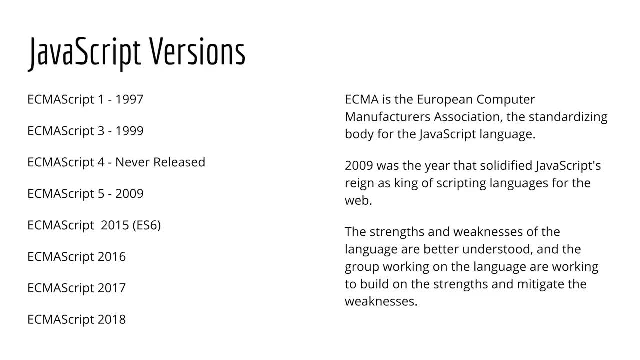 other programming languages that we are already familiar with and comfortable with. And Douglas Crockford really stepped in and said: you know, wait, look, JavaScript is its own language and it has its own powerful features in its own right And if you understand it and make use of that power, 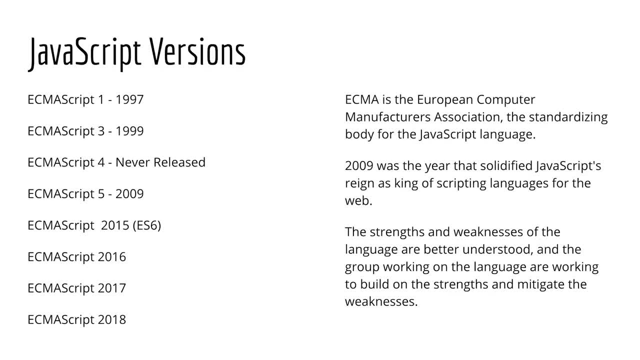 then it really is valuable to keep it the way it is, And it took a while for him to convince people of that, But in 2009, they released ECMAScript 5, and ECMAScript 4 was scrapped. They started to go a different direction entirely, and then they 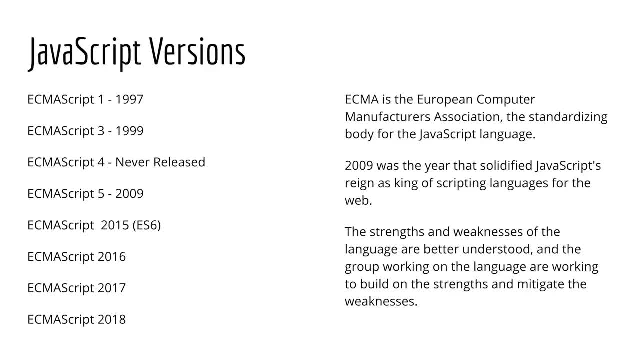 scrapped that direction entirely, And so they released ECMAScript 5 in 2009.. And this is the version that, when it was released, everybody had kind of come together around the table and said: JavaScript is going to be the scripting language for the world. 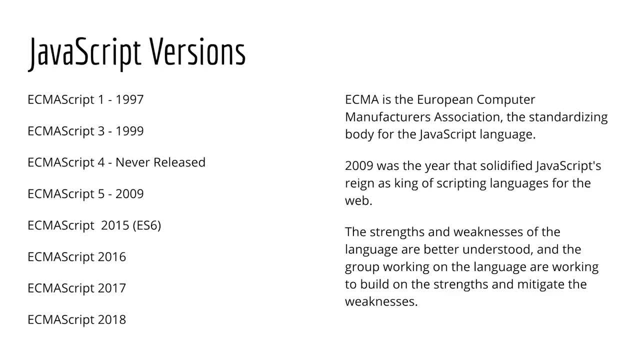 And because everybody had agreed with that. this is when JavaScript really took off and made it past its troubled beginnings, and its difficult beginnings was here in 2009.. In 2009 is when JavaScript became king of the web, because all of the major players agreed this is going to be the 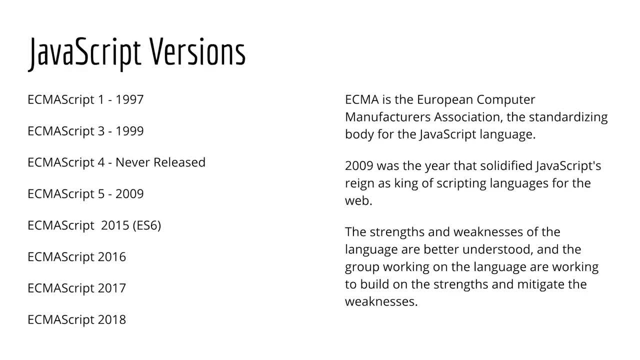 scripting language, the programming language of the web, And they built in a lot of features. There's a lot that's built in. There's a lot that's built into ECMAScript 5 that we'll be using throughout this course Over the next 10 years. there was a lot of work on JavaScript And they really wanted to move it. 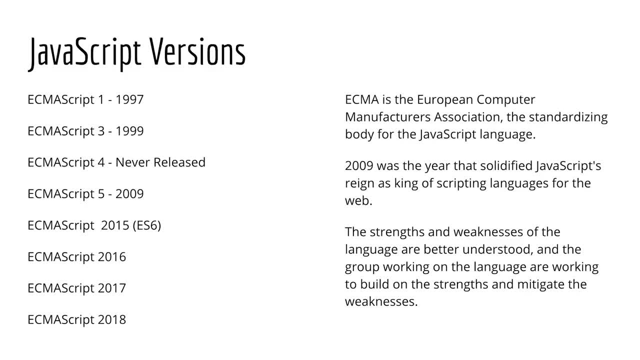 from being a scripting language to a general, all-purpose language, something that was very powerful, And in 2015,, ES6, what is commonly referred to as ES6, was released. Sometimes it's called ECMAScript 2015.. Those two terms are interchangeable, But ES6 was released and it's a 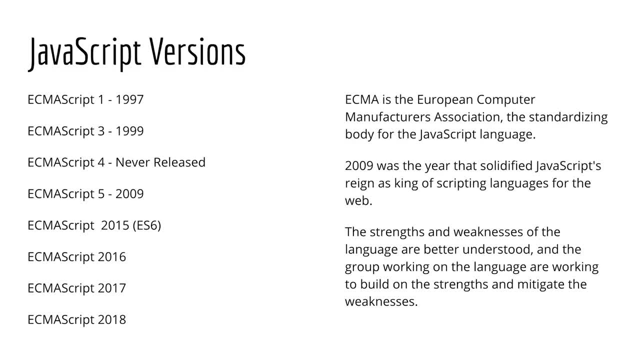 big release. A lot changed and a lot was added and a lot of JavaScript was made more powerful and it turned into a more general all-purpose programming language, And a lot of what you'll be learning in this course are pieces from the 2009 ECMAScript 5 standard. 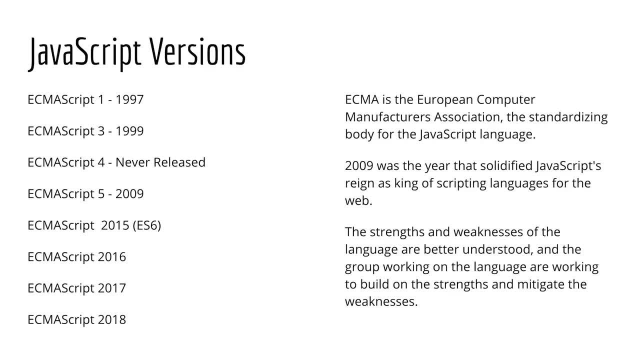 and pieces from the 2009 ECMAScript 5 standard, And a lot of what you'll be learning in this course are pieces from the from the ECMAScript 2015 ES6 standard together, which really make up the major part of JavaScript. 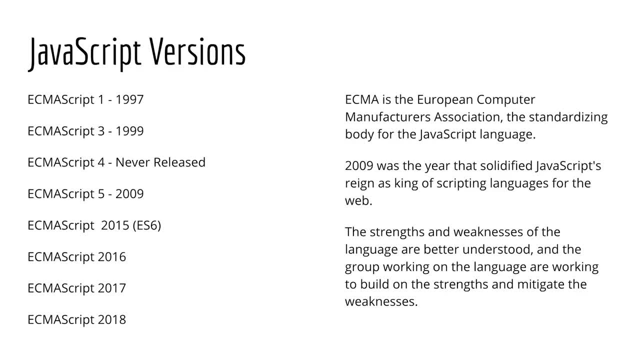 Since 2015,. the standardizing body has been in a nice cadence of releasing new versions each year And from then on, instead of calling it ES7 and ES8 and that kind of stuff, they stuck with the year. So they came out with ECMAScript 2016,. 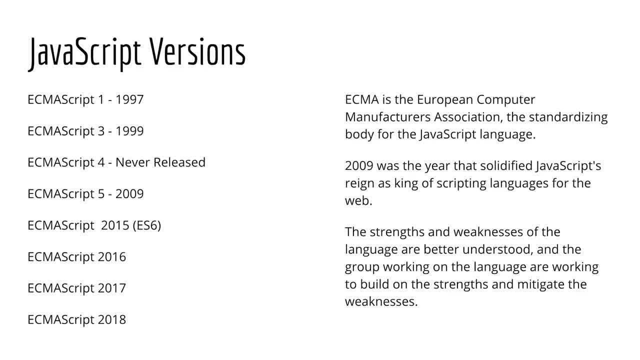 ECMAScript 2017, and so on and so forth, And each year there are smaller new additions added, but on the whole these additions are fairly small and there'll be more advanced pieces that we won't see nearly as much of in this course. 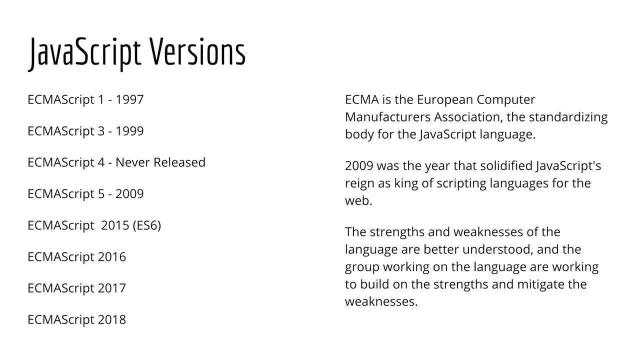 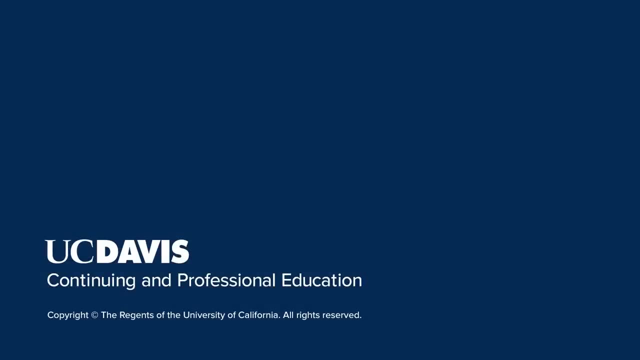 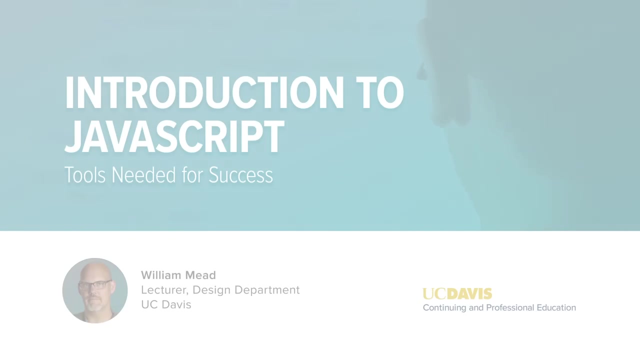 because this is a beginner's course, but we will be doing a lot with ECMAScript 5 and ES6 or ECMAScript 2016.. So dive in and I hope you enjoy learning about JavaScript as we go along here. Tools and skills needed for success for learning JavaScript. 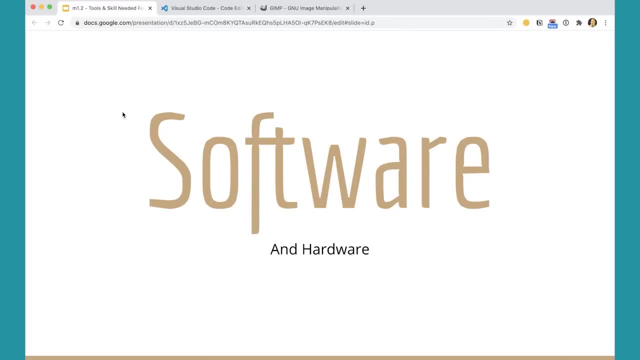 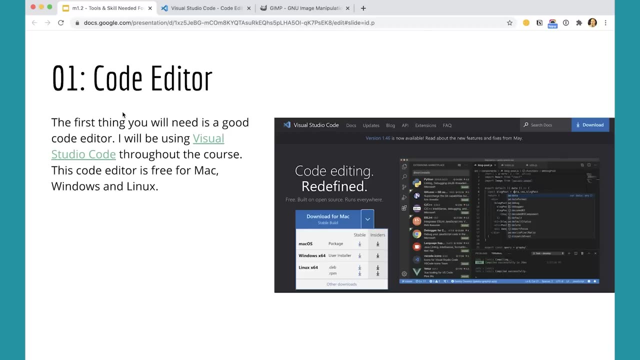 First we'll talk about software and then we'll talk a little bit about hardware. The first thing you're gonna need in order to work with JavaScript and write JavaScript is a good code editor, And I recommend using Visual Studio Code not to be confused with the Visual Studio product. 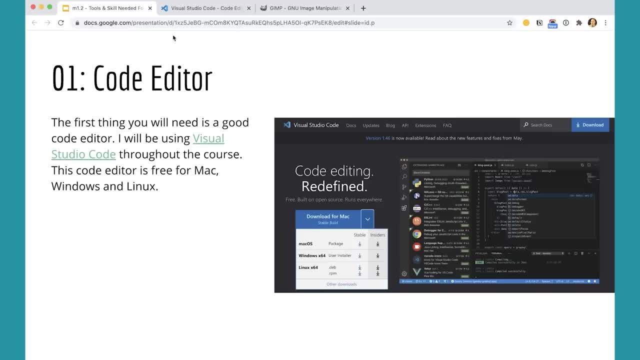 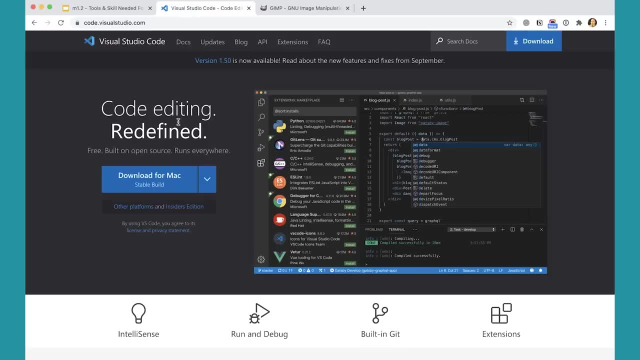 but Visual Studio Code And I have that in this browser tab here and you can download that for Mac or for Windows or, I believe, also for Linux. you can get Visual Studio Code And it's a really good code editor. It's very popular these days. 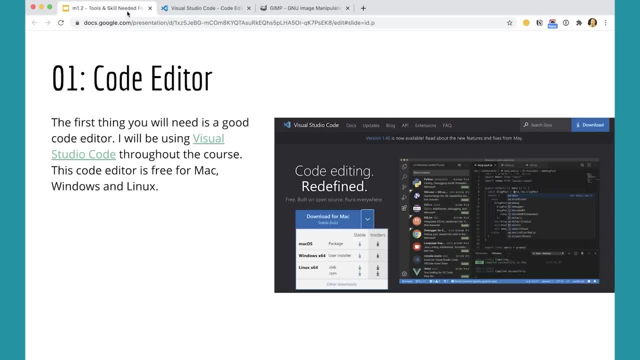 There are plenty of other code editors, but if you have other code editors out there, you could use Atom, you could use Sublime Text. Even if you have Dreamweaver, you could use that as a code editor. Dreamweaver has a lot of other stuff built into it. 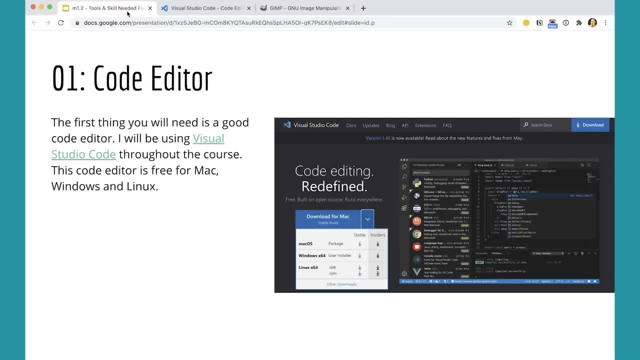 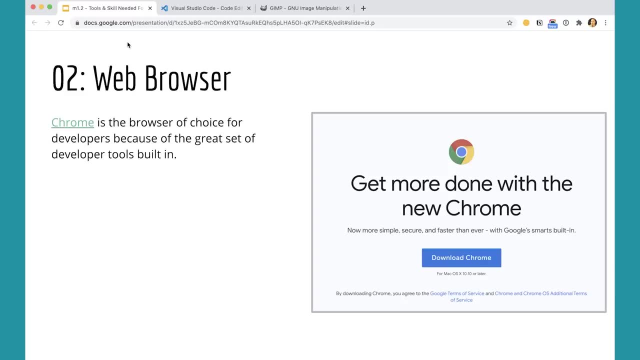 that you don't need, but it works perfectly fine as a code editor, if you wanna use that as well. The second thing you're gonna need is a web browser, And I'm gonna recommend that you use Chrome. Chrome has A lot of the developer tools that developers use. 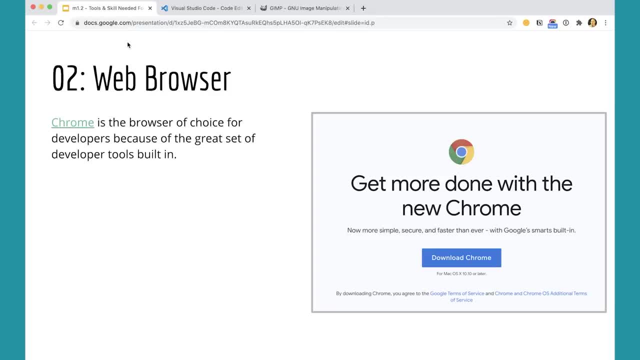 they're built right into Chrome and they're easy to access. You can also use Safari or Firefox or Microsoft Edge, or Brave is another browser out there- But- and there are other browsers out there as well- And many of them also have developer tools. 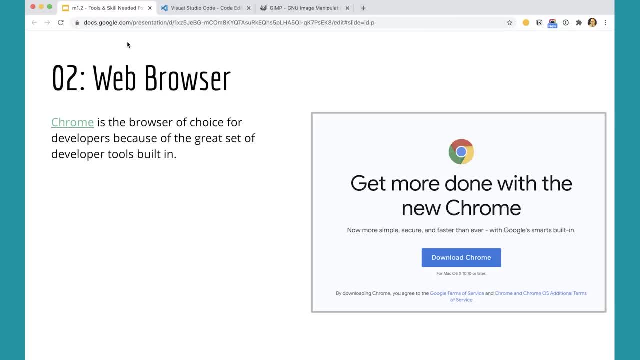 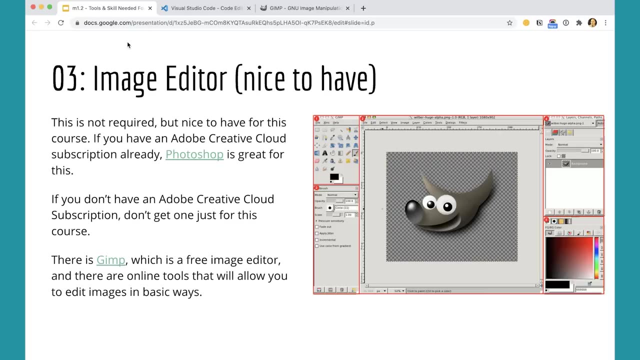 but most developers use Chrome and get comfortable with the Chrome developer tools, So I recommend that you download Chrome and use that browser. You're also gonna need an image editor And if you have access to Photoshop, that's great. Photoshop is fantastic for this kind of thing. 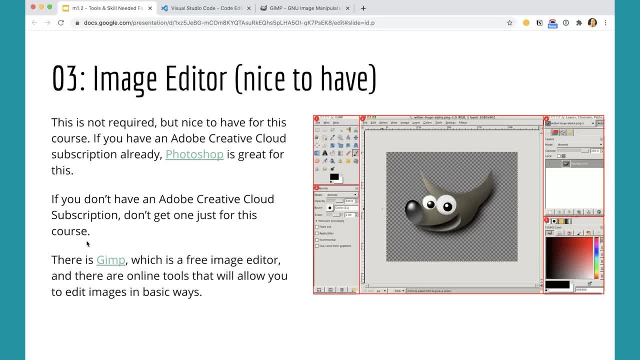 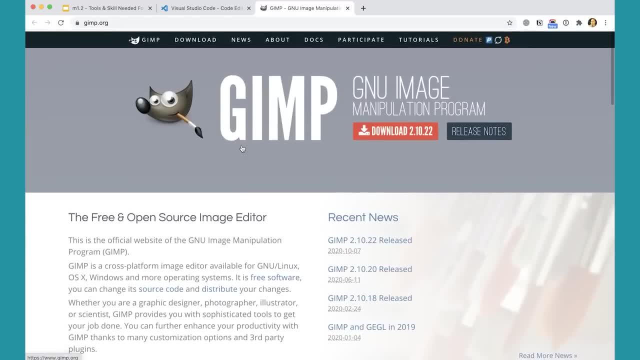 But if you don't have access to Photoshop, there's another one called GIMP which is free And you can go download GIMP and I have that pulled up here So you can actually download GIMP for Mac or for Windows and that kind of stuff. 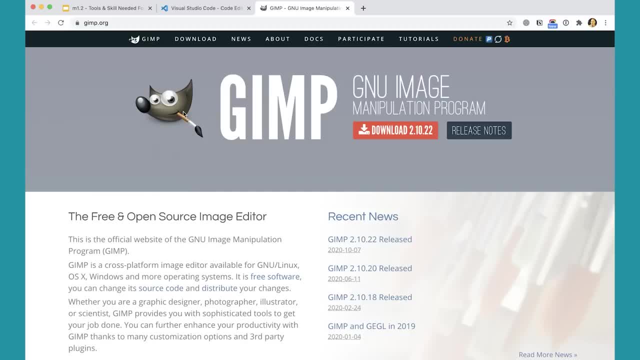 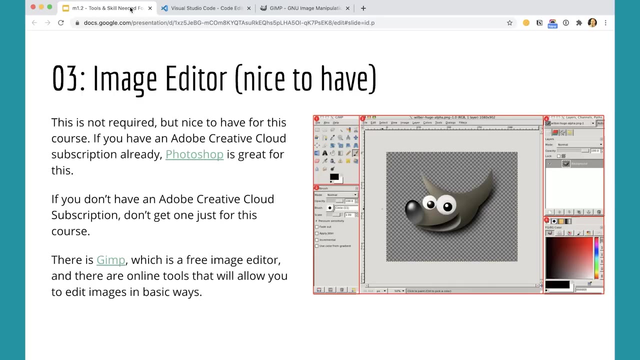 There are also online tools, web pages, that will allow you to upload your image and optimize it for the web and do some different kinds of image editing right through your browser. So you might find some of those types of tools as well, But you will need some sort of image editor. 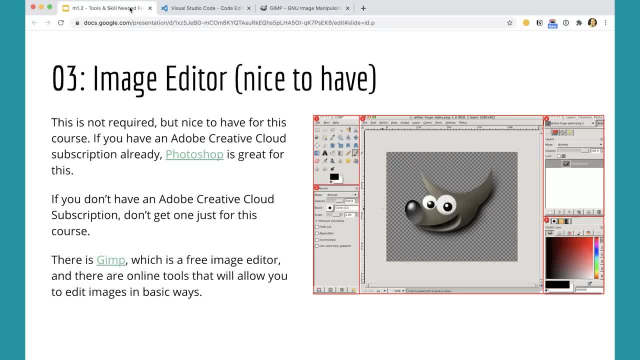 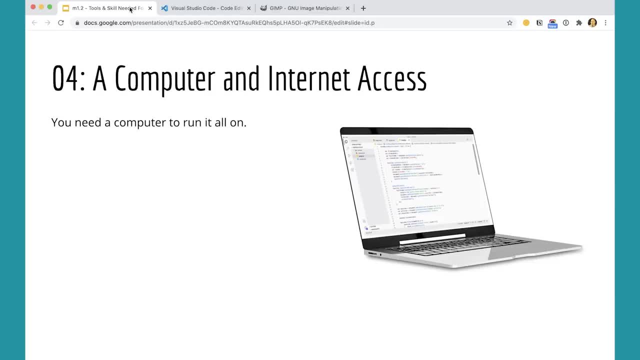 to help you with working with images. That's kind of a nice to have. It's really. it's not absolutely necessary, but it's really nice to have. Next, you're gonna need a computer and internet access. It may sound obvious that you're gonna need internet access. 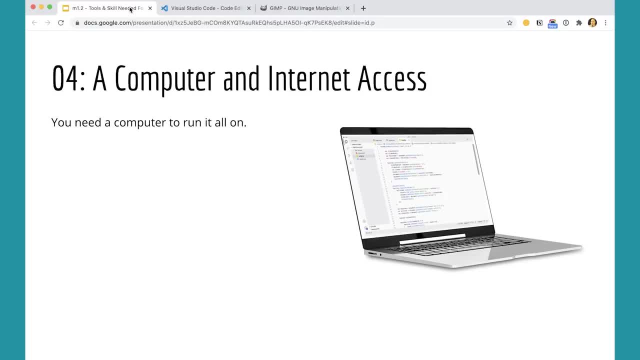 to do an internet class, but you are gonna need that And you will need a computer, whether it's a laptop or a desktop. What's not gonna work very well is either a Chromebook or a tablet or a phone. You're really gonna need something. 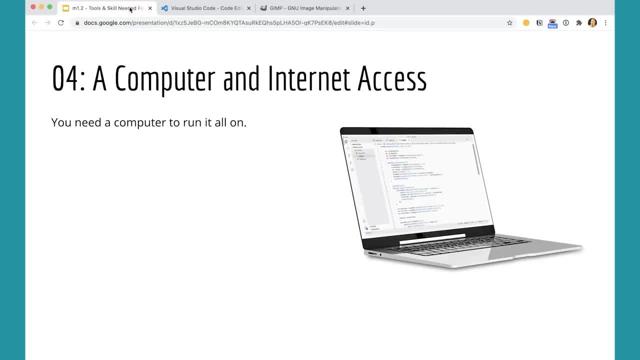 that you can write code on and save files to, And iOS is not. you can make it work, but it's not really up to the task. You'll be fighting it every step along the way. So you wanna be working with Mac OS X. 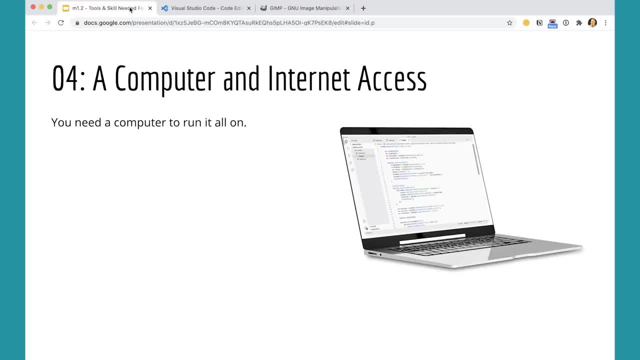 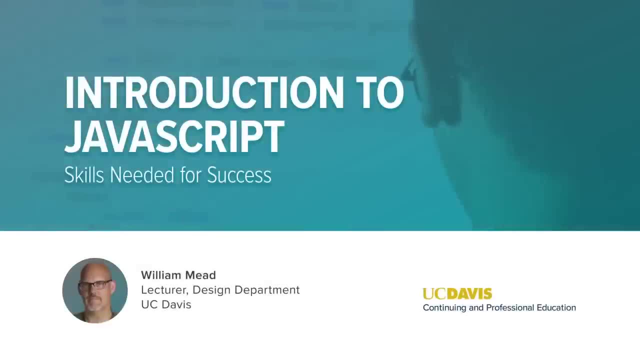 or Windows 10 on a computer in order to really make this work. Let's talk about some of the skills that you need to be able to do this. Let's talk about some of the skills that you need to be able to do this. 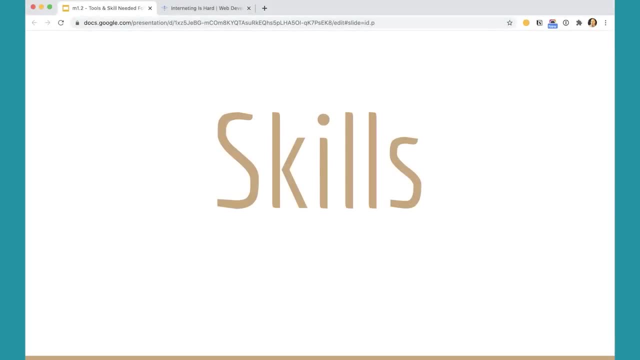 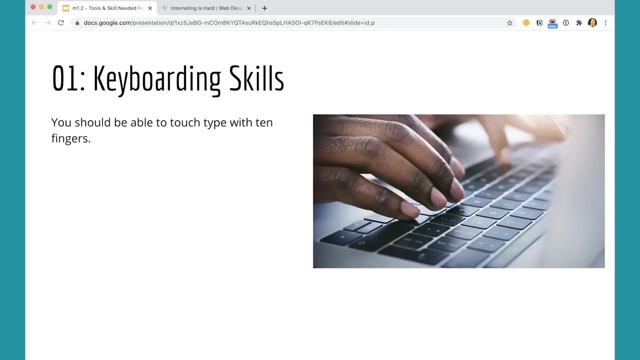 Let's talk about some of the skills you need in order to be successful learning JavaScript. First and foremost, you need to be able to type, And by typing I mean typing with 10 fingers without looking at your fingers. touch typing, And it will really help you to be able to do this. 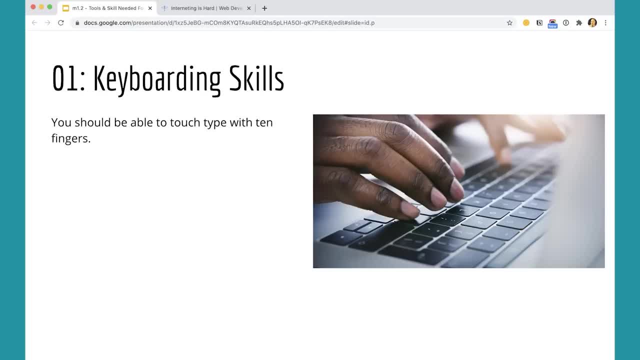 If you're somebody who hunts and pecks with one finger or two fingers, you may be pretty fast at it, but it really will slow you down for programming, And so I recommend that you do some online typing programs. There's plenty of places online where you can learn how to type. 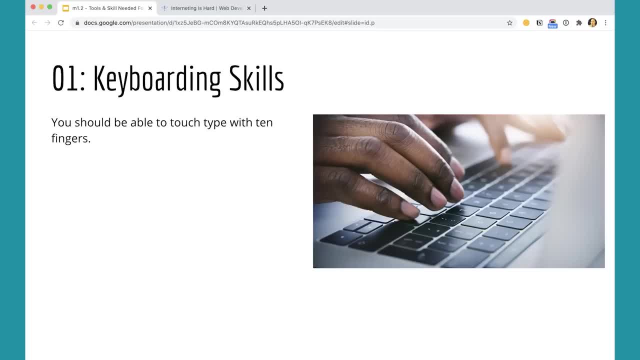 You don't have to be terribly fast at typing, but you do need to be accurate. Or if you're not accurate with typing, you have to at least stop and go back and fix every single error, And I have known a lot of students over the years. 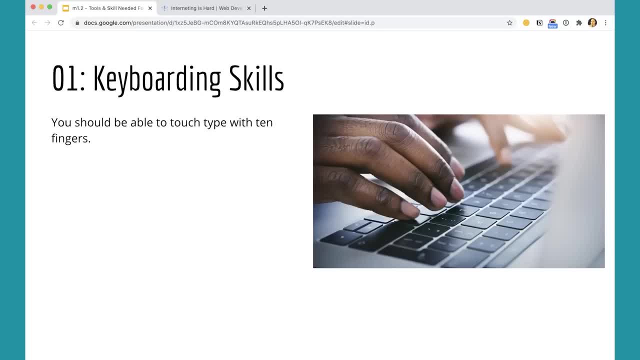 that struggle a lot with typing and it really impedes their ability to learn something like JavaScript. So I really recommend that you get those keyboarding skills if you don't have them already. The second thing that you need is you need to be able to manage your files. 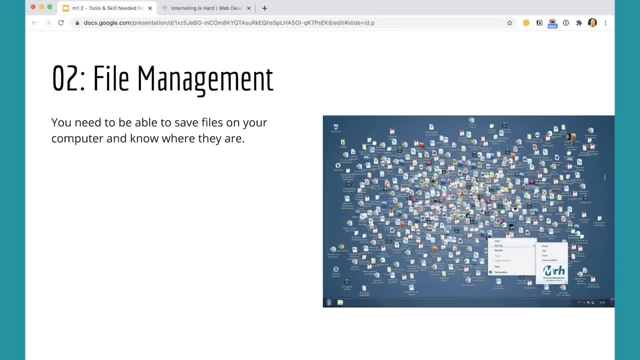 That means that when you save a file in your computer you know where it is, not just going into the file menu and choosing the most recent files thing. If that's what you do to find your files, then you need to really get good at file management. 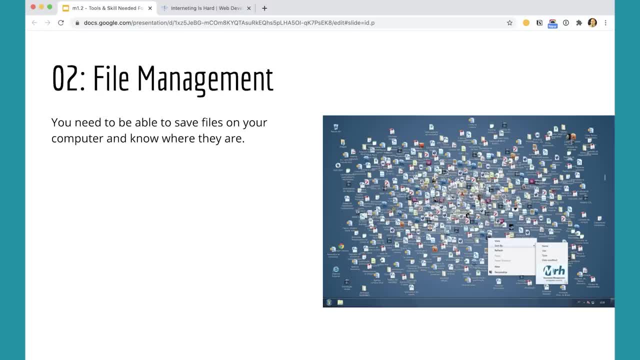 And if your desktop looks like the picture here, then you're gonna be in trouble. Make sure you're comfortable with saving files into folders and you know how to do that and where those folders are. On the web, everything is linked, So if a file cannot be found, 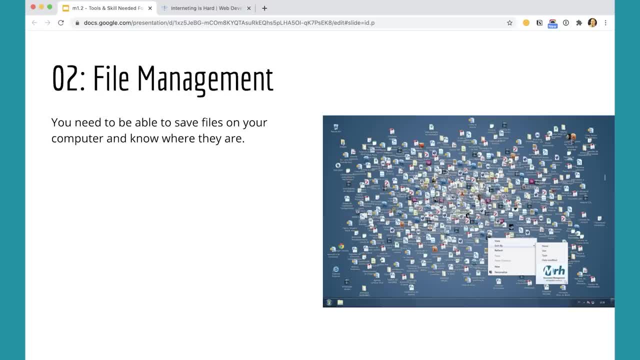 if a file's not in the right place, then your project will break, and we don't want that to happen. So make sure you clean up all of your files and work with a clean desktop, And for every project you should have a folder. 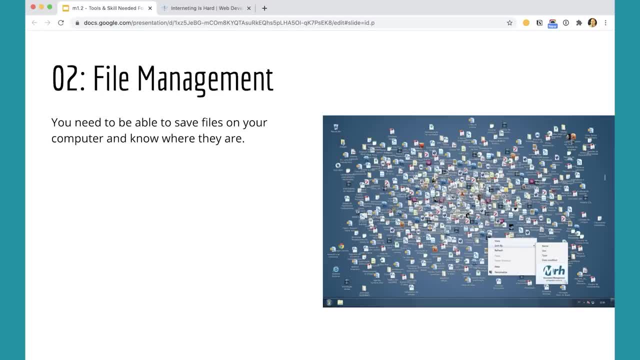 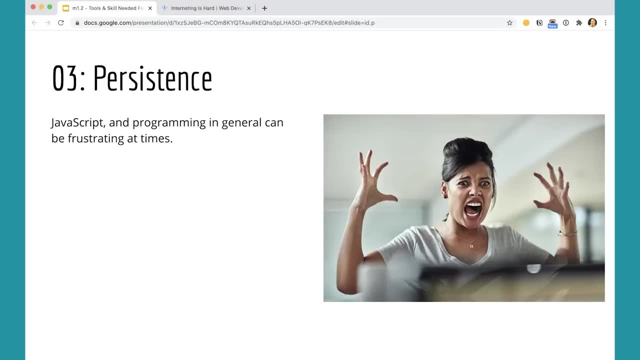 and all the files you need for that project should be in that folder. The next thing that you need is persistence. Learning JavaScript is not easy. it's challenging, And maybe that's true for every programming language, but JavaScript in particular is. it's got some quirks to it. 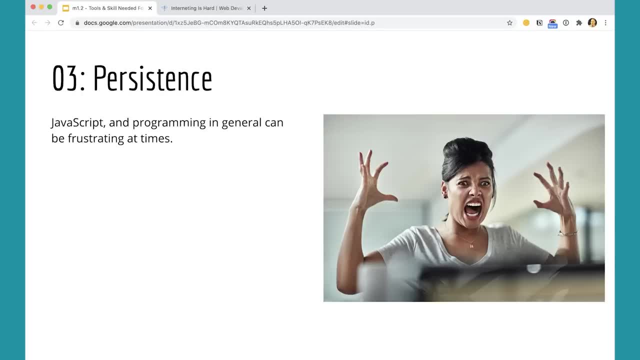 and it takes some getting used to, And there will be times when you're frustrated when things aren't working the way you think they should and you just need to take a break, step away from it and then come back to it. 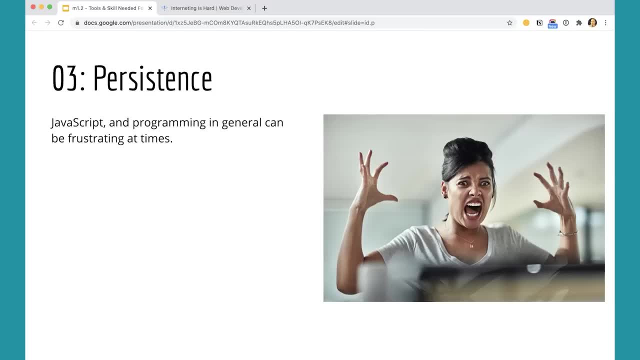 But come back to it because it's worth learning And even though it's hard, it's definitely worth putting in the effort and being persistent to get there. I have told many students over the years: if you're not banging your head against the wall, 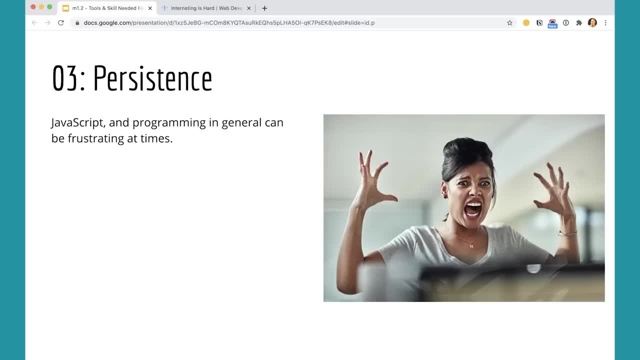 you're not learning JavaScript. All my students will tell you that. I say that over and over and over again, And it's frustrating, especially in that moment when you realize you just left that one character or a semicolon or something like that and that broke the entire script. 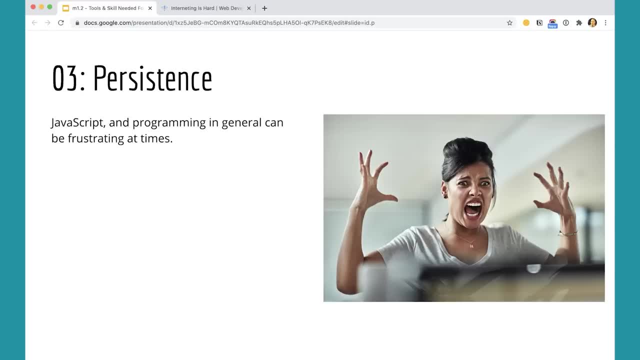 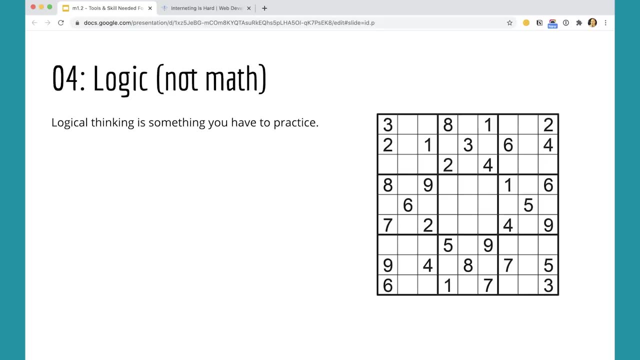 But stick with it, keep working at it, stay calm, keep pushing forward, and you'll make a lot of progress with it, I promise. The next skill that you need is to be good with logic, And logic is a learned skill. 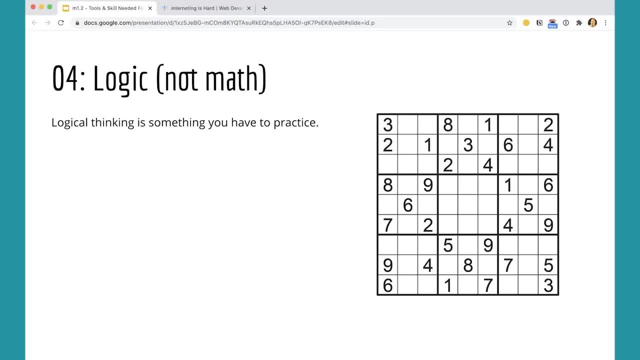 Some people are naturally very logical, but it's something that you can practice and develop, And there are lots of tools and games out there that will help you build your logic skills. Sudoku is a great place to go for puzzles that will help you build your ability to use logic. 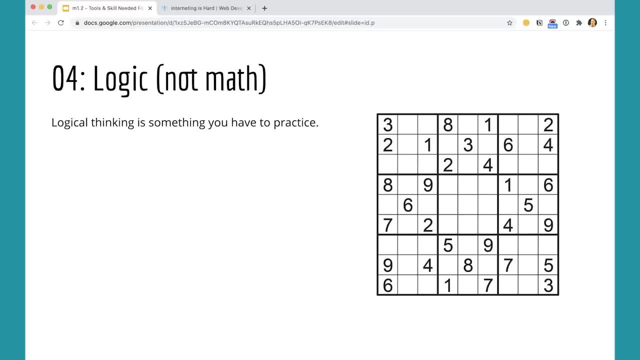 Programmers often use a lot of logic skills. You can use math as well, but math is not that important to begin with. It's really the logic skills that you need. You might need some basic arithmetic, but I don't do a lot of programming. 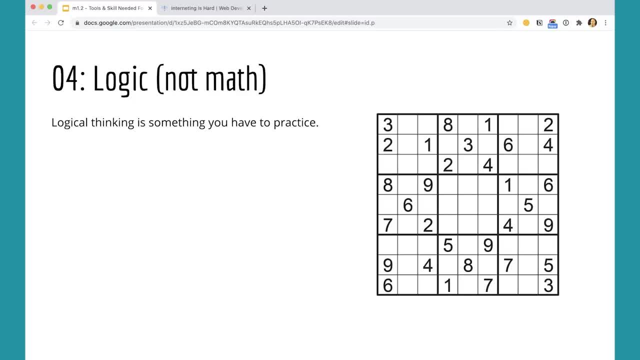 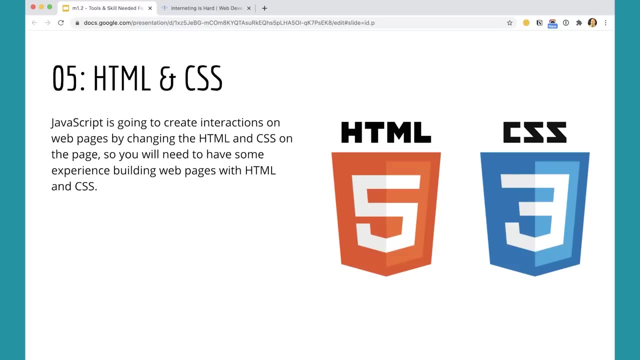 that involves very sophisticated math and a lot of programmers don't. There are programmers that do, but we don't need that in order to get good at JavaScript, But you do need to be good with logic. The next thing is you really should know HTML and CSS as well as you can. 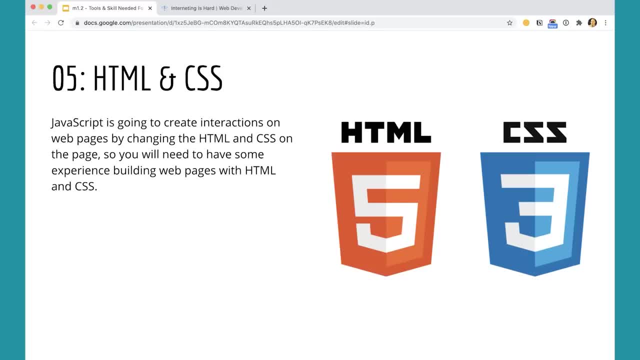 JavaScript manipulates the HTML and CSS that makes up the page. That's how it works, That's what it does, And if you don't know HTML and CSS, you don't really know what you're manipulating. So I recommend building some skills with HTML and CSS. 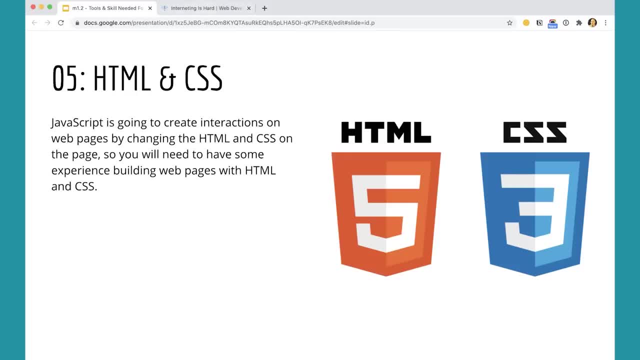 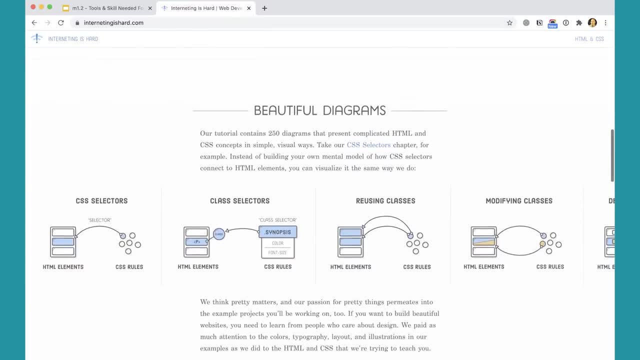 if you don't already have them, And a good place to go is this. Internetting is Hard. website here. This is a really great tool. It's a tutorial. They've got a lot of really great. it's very simple the way they've explained things. 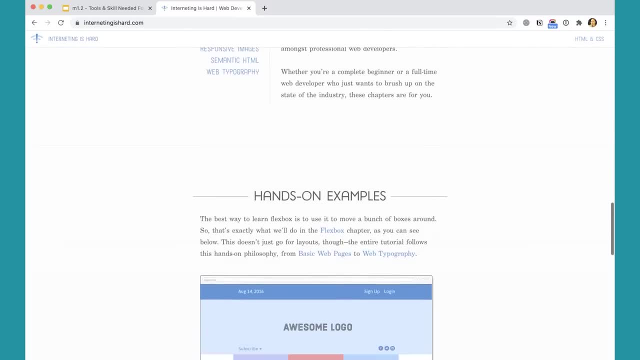 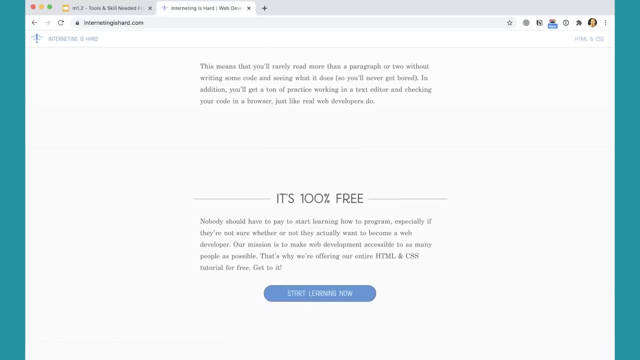 and they've got a lot of great examples and tutorials here that will help you with learning HTML and CSS- and it's free, So I recommend going and looking through the Internetting's Hard website if you need to get caught up on HTML and CSS. 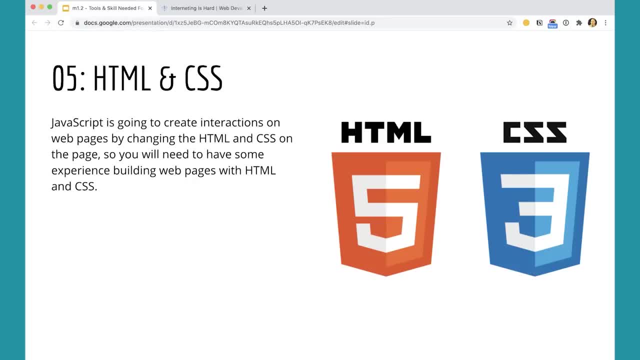 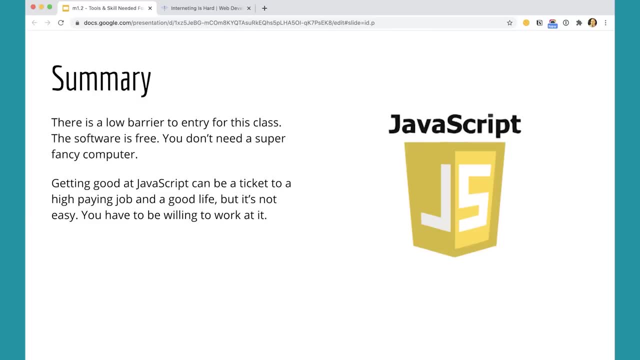 Or if you've never done any HTML and CSS at all, then maybe take a course in HTML and CSS before before diving into JavaScript. In summary, there's a low barrier for entry to this class. The software is free. You don't need a super fast or super fancy computer. 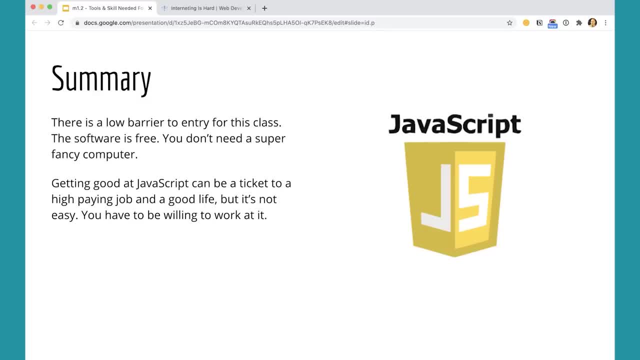 And getting good at JavaScript can be a ticket to a high-paying job and a good life, But it's not easy. You're going to have to work hard to get there, But it really is worth it if you keep working at it, And I hope that you continue with us. 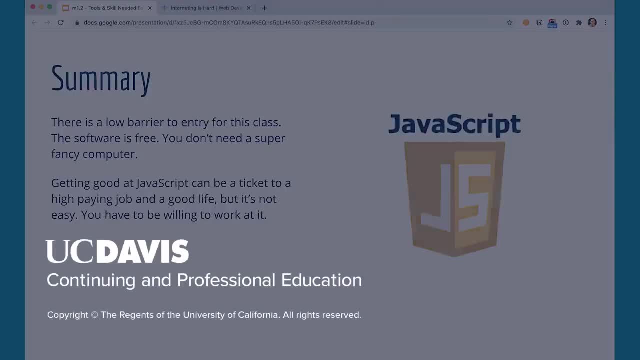 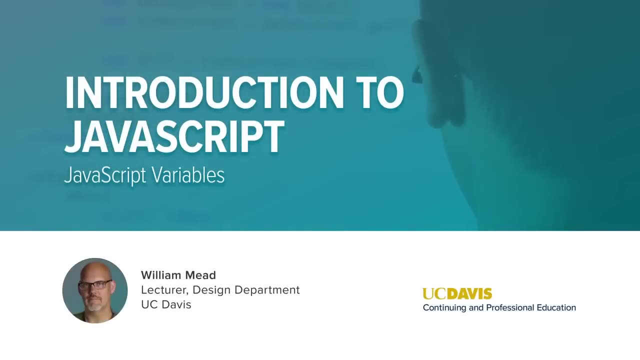 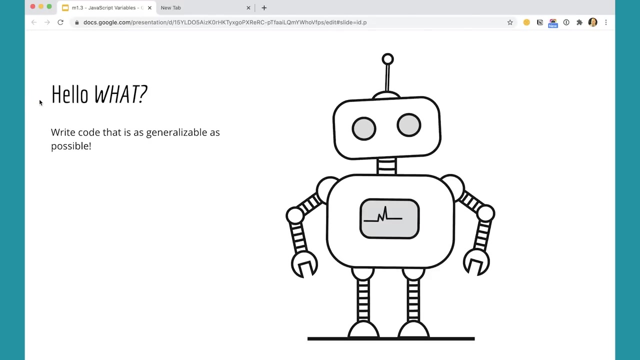 and see all the cool things that you can do with JavaScript- JavaScript Variables. It's good practice when programming to write code that is as generalizable as possible. It allows the code to be reused and helps limit the effort of writing and maintaining redundant code. 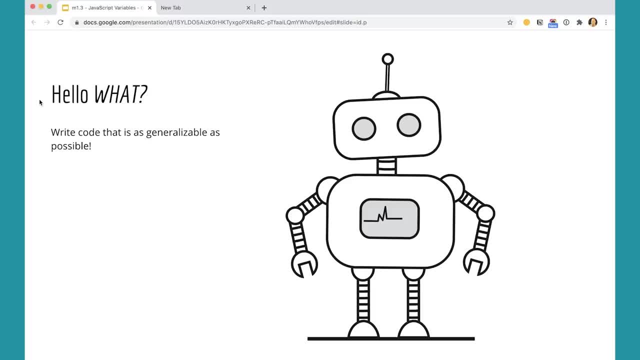 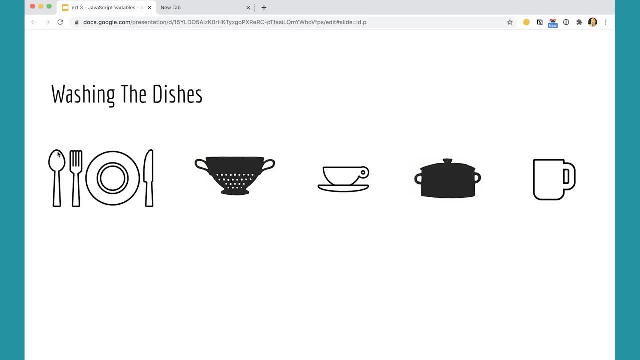 Imagine somebody gave you a robot as a gift to do chores around your house. You have to teach it how to do your chores. What if you wanted to teach it to wash the dishes? That would be great. It would be really helpful to have a robot wash the dishes for you. 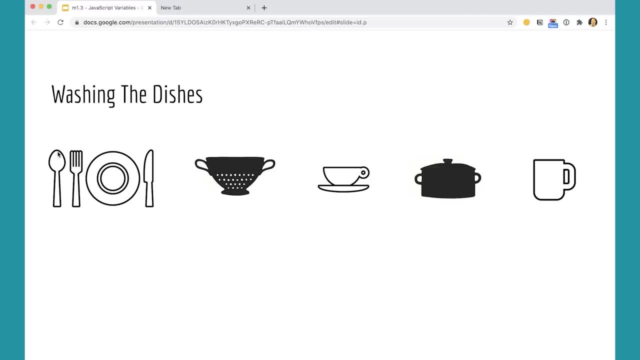 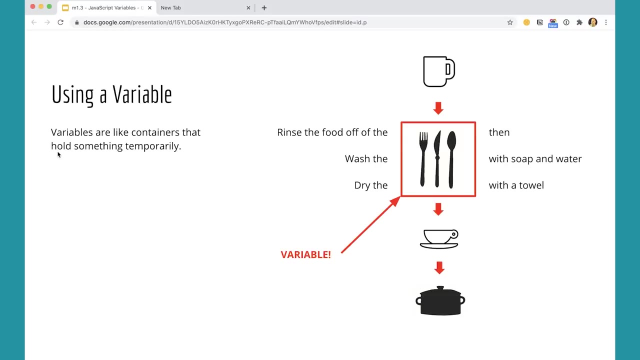 But what if you had to write different instructions for each dish in your house? That would be a lot of dishes and perhaps a lot of instructions, And that wouldn't be so great. What we can do with the variable is that we can treat it as like a container. 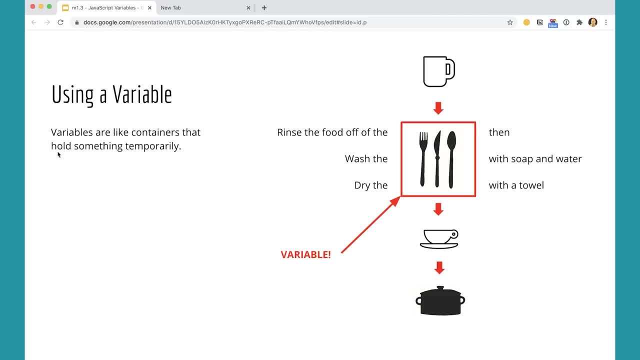 And then we can write a set of directions and pass each item through that set of directions. So here in this diagram currently we're going to rinse the food off the silverware and then wash the silverware with soap and water and then dry the silverware with a towel. 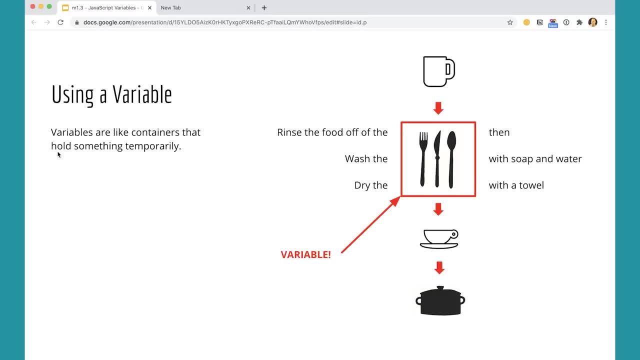 and then move on to the next item, Which perhaps might be a cup. The box, the red box that you see here, is really the variable. It's a temporary container that we can pass these items through, and we can teach our robot to wash all of the items. 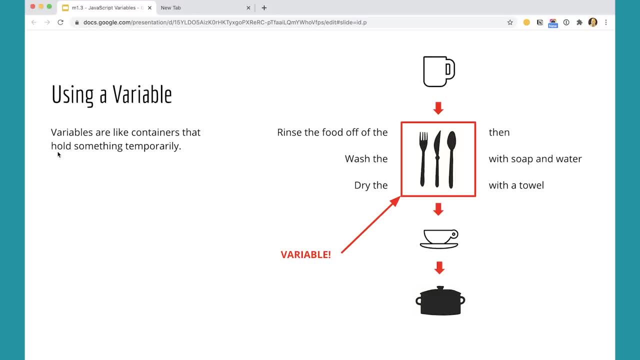 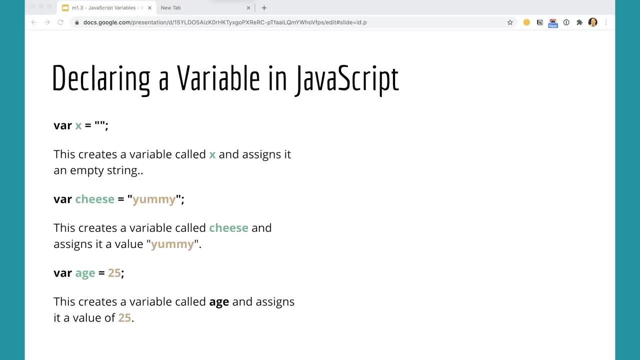 one at a time using this container, And that will make your instructions more modular and more reusable, And that's really helpful. So let's talk about some ways of declaring a variable in JavaScript. We'll start with one of the most basic ways. 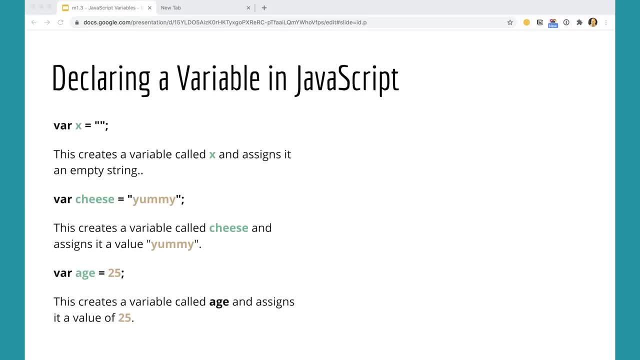 which is using the var keyword V-A-R. So here I have a variable called x. I'm creating and JavaScript will then recognize x as a variable and I'm assigning it an empty string. two sets of quote marks there, followed by a semicolon. 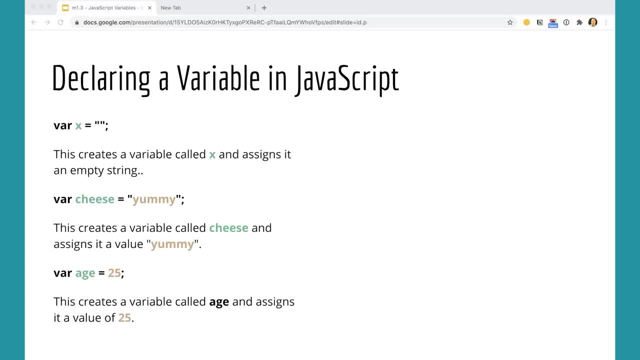 And that means that variable x holds an empty string. On the next example, we're going to use a variable that holds an empty string. For example, I have a variable called cheese that I've created and it's holding a string called yummy. 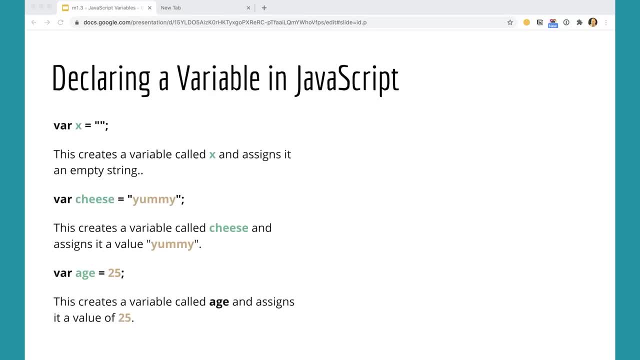 The equal sign here is an assignment operator. It means assigned, So yummy is assigned to cheese. It's easy to use the word equals because we're used to seeing the symbol in association with math, where we see two plus two equals four and we say equals. 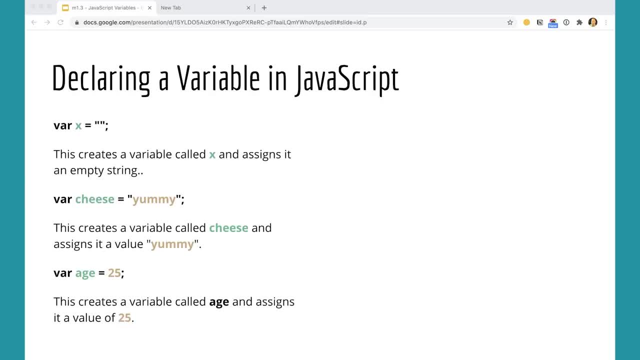 But in programming we want to say assign- Yummy is assigned to cheese. And then the next example: we have a variable called age and it's assigned a value of 25.. 25 is a number. It doesn't need to go inside quotes. 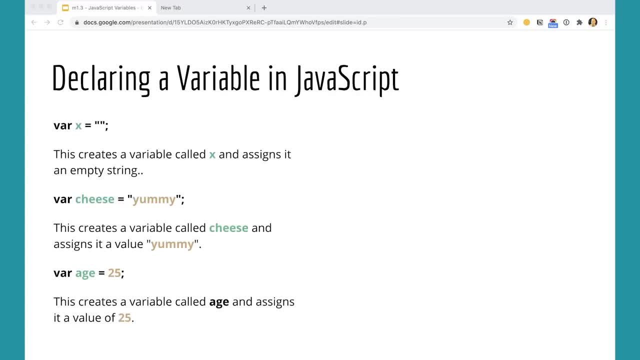 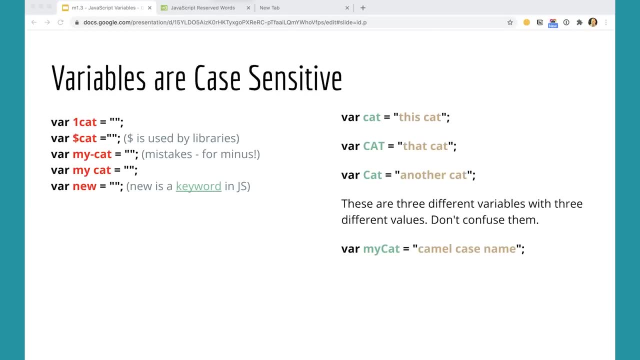 because JavaScript knows what a 25 is. In JavaScript, variables are case sensitive and they have to follow certain rules. For example, a variable has to start with a letter. You can't start with a number. So this variable over here that says one cat is not going to work. 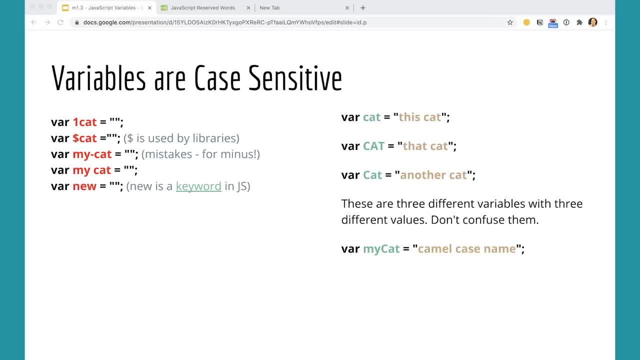 because it starts with a number. Also, you should not start variables with something like a dollar sign. They're used a lot by libraries, so you should not do that as well. The third example: my dash cat is not going to work because JavaScript sees the dash as a minus sign. 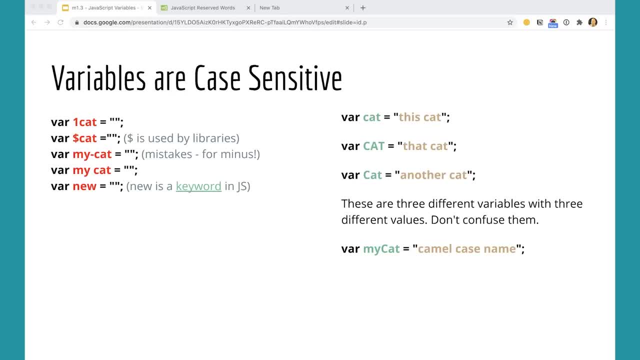 So it thinks you're trying to subtract cat from my, which is not going to work. It's not going to work at all either. Also, you can't have a space in a variable name, because var my might be a variable, but then it doesn't know what to do with cat. 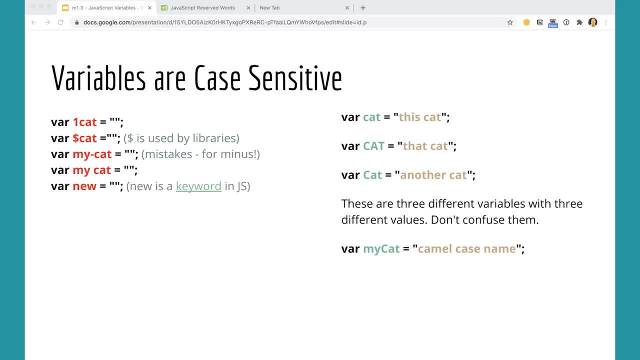 because it sees that as a separate thing, because there's a space in there. And then, finally, there are certain keywords in JavaScript that you can't use as names of variables, like new is a keyword, And over here I have some of the keywords pulled up. 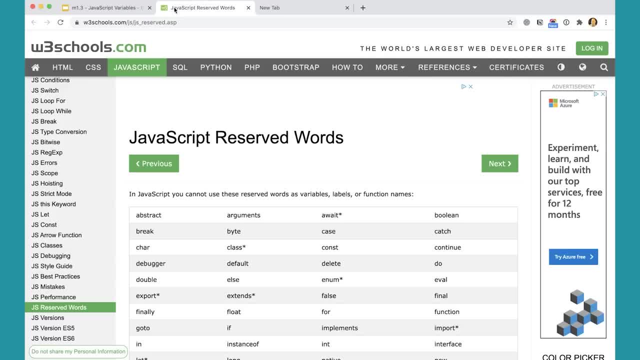 on the W3Schools website. W3Schools is one of the places you can go to get a lot of information about JavaScript- basic information. We'll also look a lot at the MDN, the Mozilla Developer Network, which is really the most authoritative place. 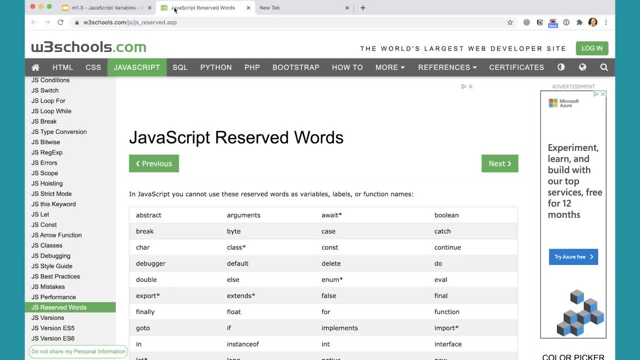 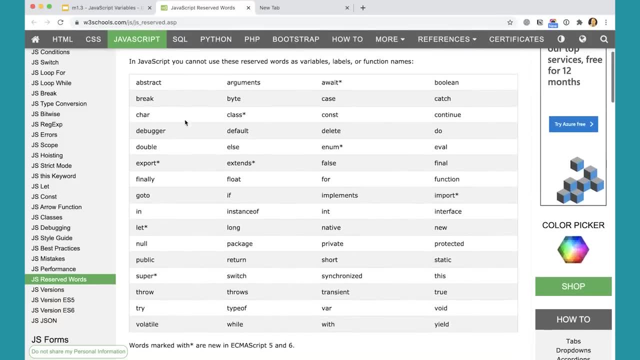 to get information about JavaScript, but it can be a little bit overwhelming at first as well. But the W3Schools is a little bit easier to understand. You can see here that there are a bunch of keywords and you'll notice that some of them have an asterisk. 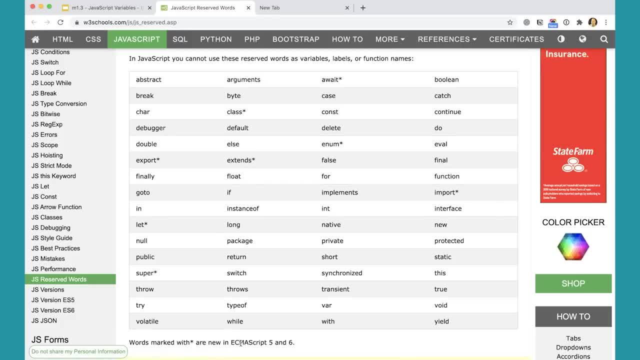 some of them don't have an asterisk in here. Words marked with an asterisk are new in ECMAScript 5 and 6.. Remember, we talked about the versions of JavaScript, So now when you see ECMAScript 5 and 6,. 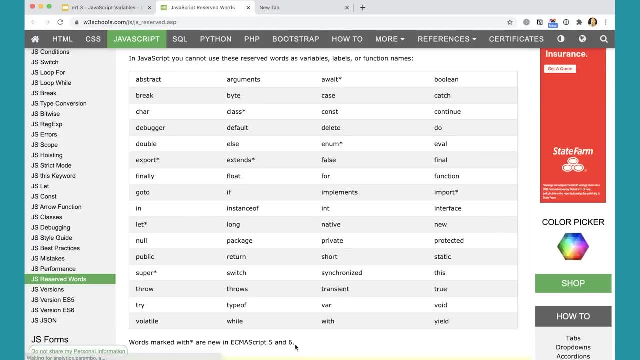 you know that we're talking about ECMAScript 5,, which was released in 2009.. That was the big release then, And ECMAScript 6, or ES6, was the version that was released in 2015.. Okay, so these are all keywords that you can't use. 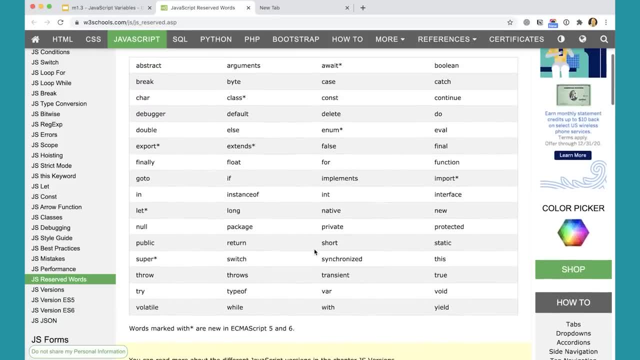 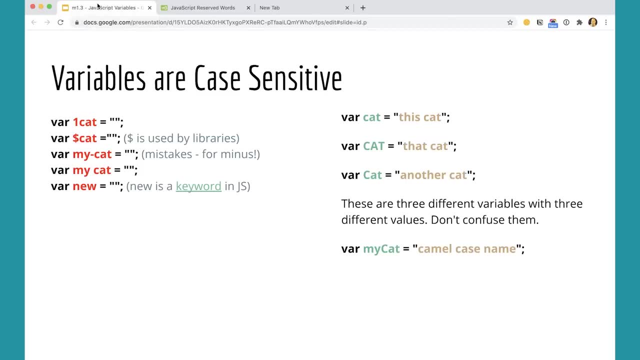 as names for variables in JavaScript. Over on the right in this image. here you'll see we have variable cat with a lowercase c, variable cat all in uppercase letters and variable cat with a capital C. These are three different variables that hold three different values. 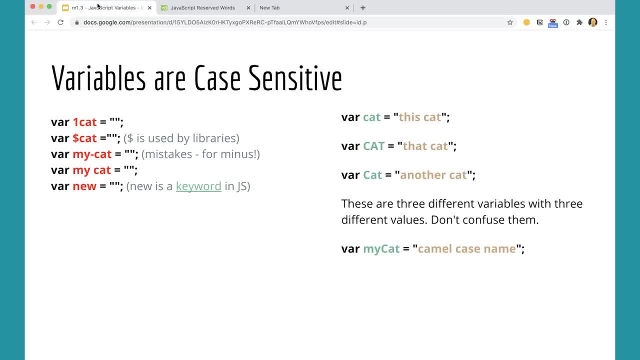 It's generally better practice to use lowercase letters when creating variables or to do what's called camel casing, like we have down at the bottom here- My cat with a capital C in the middle, So it's kind of like a hump in the middle. 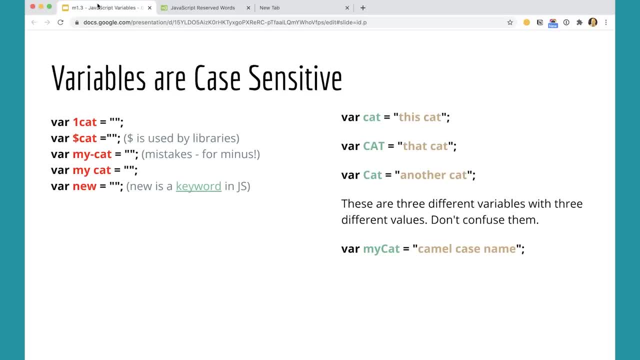 We like camels in JavaScript, So that's called camel casing. That's not specific to JavaScript, but it's something that is in a lot of programming languages But we use that frequently. in JavaScript. You'll frequently see variables that are using camel casing. 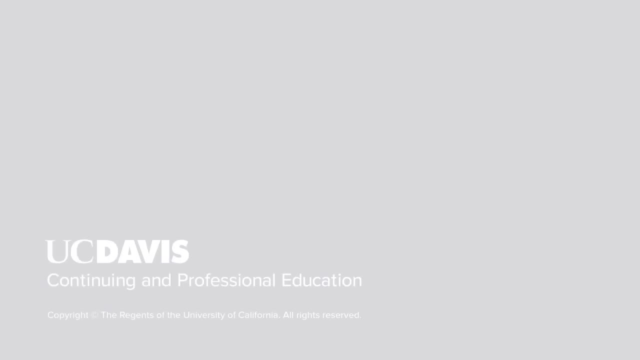 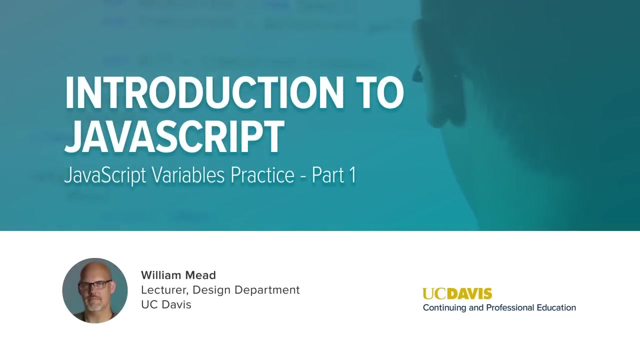 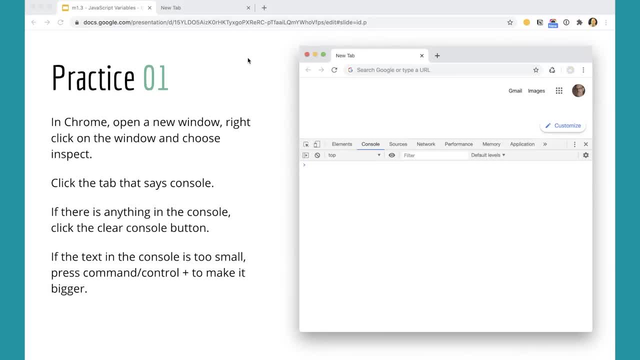 We've been talking long enough about JavaScript, So now it's time to actually get down and write something, And I hope you're ready to do that, because it's pretty exciting to start seeing it come alive on web pages- And it'll be a little while before we start making. 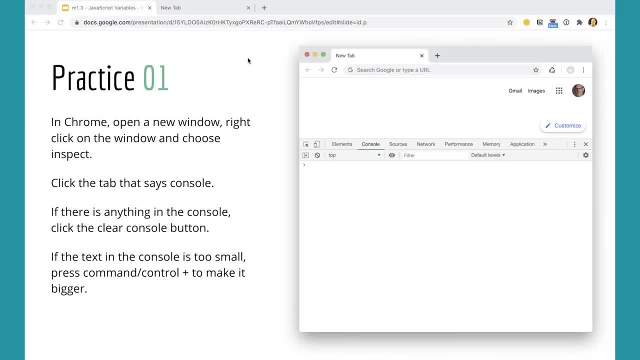 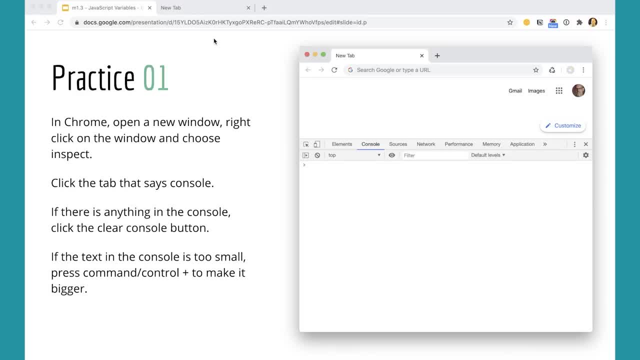 And what we can do with our browser is we can actually open just a new browser tab and use the console to write some JavaScript. Because JavaScript is native to the browser, we can write it right into the browser and it will actually do stuff in the browser. 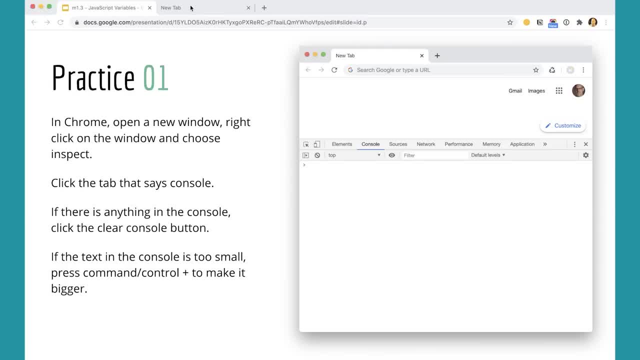 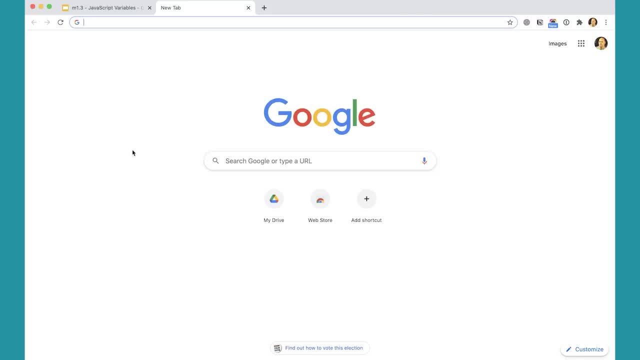 So that's pretty cool. So I have a new tab over here and you can create a new tab for yourself, And I'm just going to right click and choose, inspect, And you have to right click on the white area, Right click on an element or something like that. 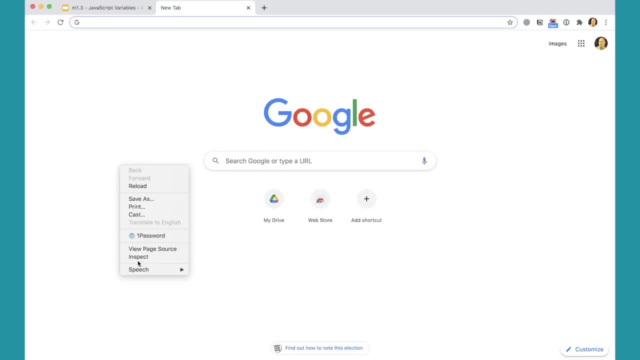 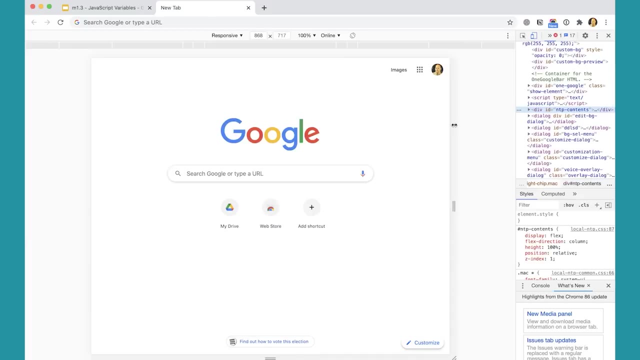 Right click on the white area and choose inspect And that'll bring up the inspector in Chrome. And again, I'm in Chrome And when I do that it might put the inspector over here. It might do some different kinds of things. 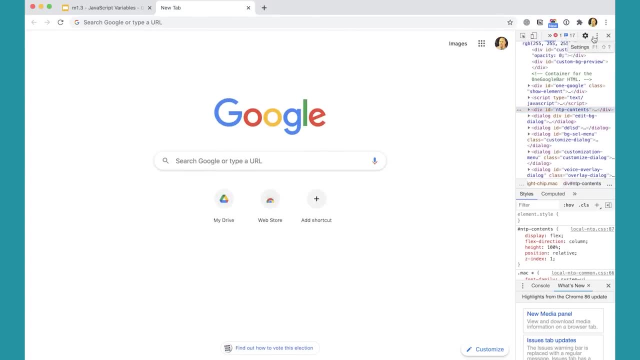 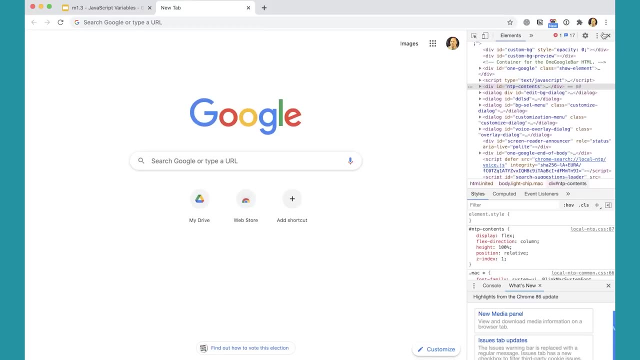 Some different buttons might be selected, But what you can do is you can use these buttons here. You can arrange this thing, make it bigger or smaller. You can use these buttons to move This inspector around. So this button here will allow me to choose. 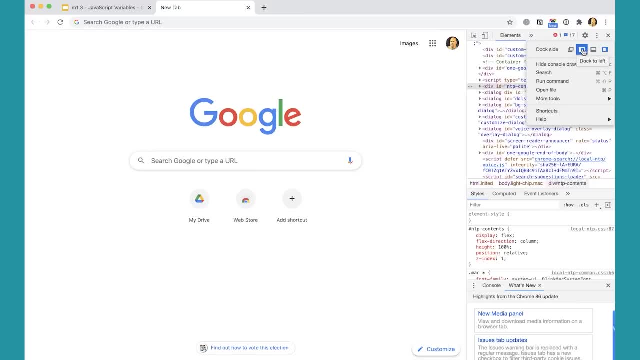 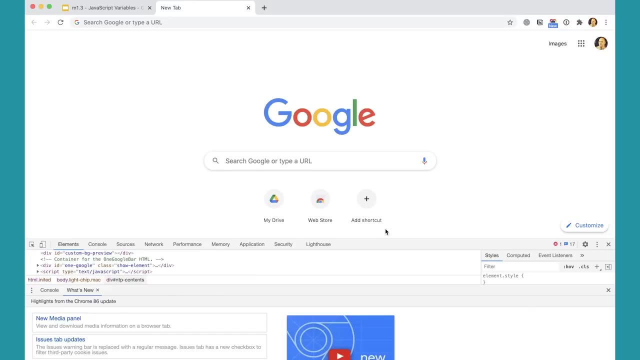 where I want it to display. Right now it's on the right, but I could put it on the left or I could put it on the bottom. I want it on the bottom in this case. Sometimes it's helpful to tear it off entirely. 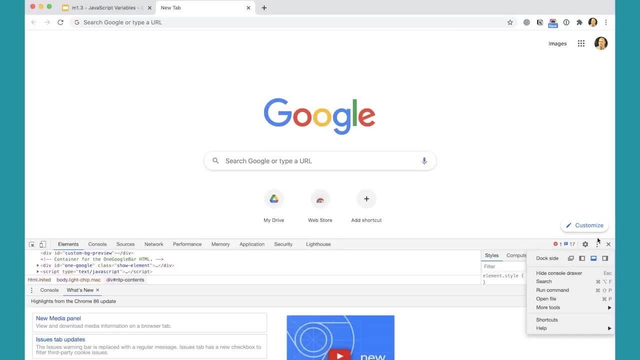 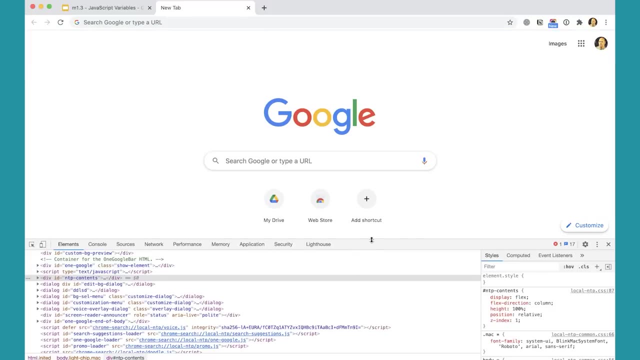 and do a different window, which is this icon, But I'm going to leave it down here on the bottom And then I want to close this thing down here because that's just giving me some information And I'm going to make this come up here. 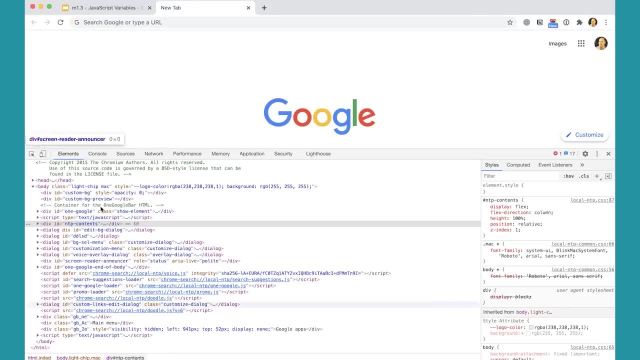 And right now I'm on the Elements tab And I can see the HTML that is making up this page And you can actually drag around on here and you'll see different elements of the page will get highlighted. But what I really want to do to write some JavaScript. 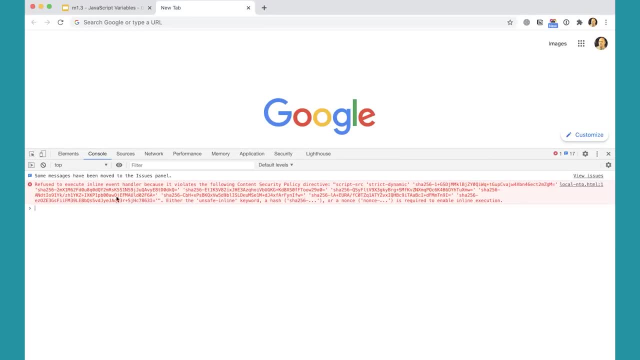 is the console, So click on the console And you'll see if there are any errors coming up or anything like that. And this is something coming over from Google right now. There's some sort of error here And I don't really care about that. 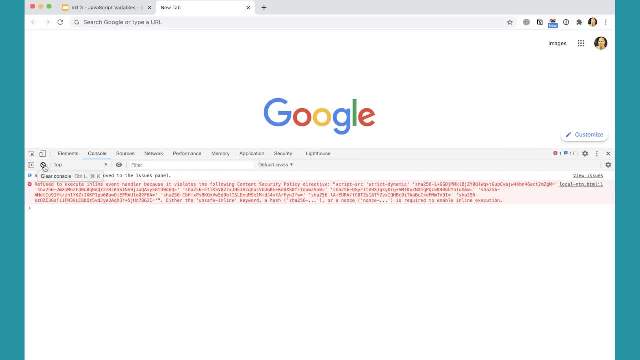 So I'm going to click on this little Clear Console button here to clear the console and get rid of that error. And now I can do things like create a variable var. cheese equals yummy And again, yummy is assigned to cheese. the variable cheese. 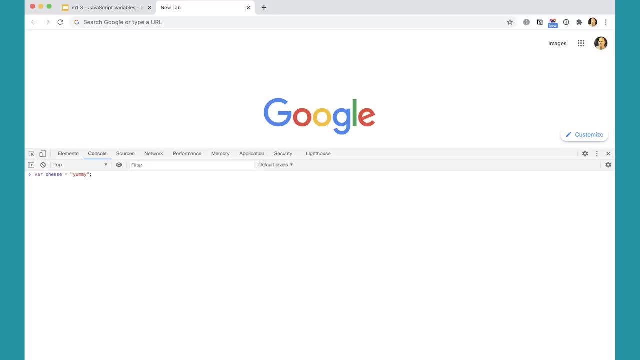 here, Put a semicolon and press Enter. Now Let's do this. Another thing that's useful is if this is seeming very small on your screen, you can use Control on Windows or Command on the Mac, the plus key to make the text larger, or the minus key. 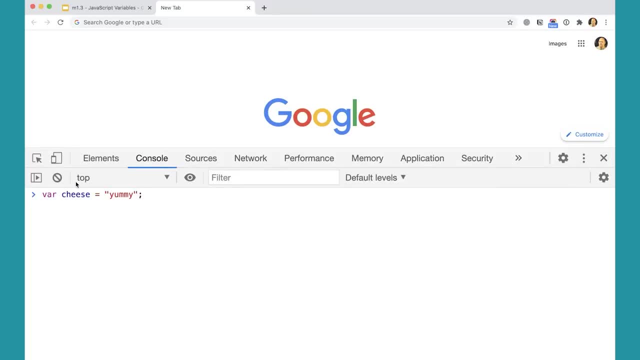 to make it smaller, plus and minus, Or you can do Command 0 to put it back to the default size. So a lot of times when I'm working with students they have trouble seeing the syntax And I recommend making the actual code larger. 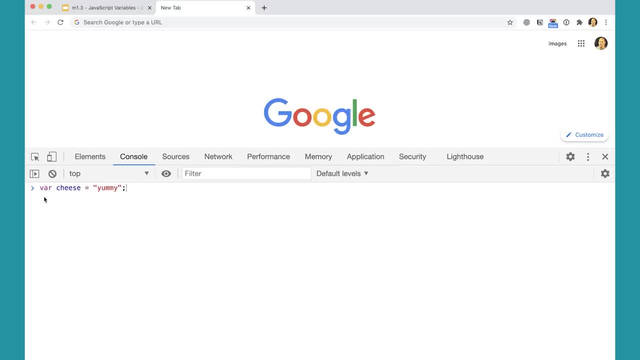 so that you can see it better. So I'm going to make it larger, like that. So var cheese equals yummy, Great. Undefined is sort of the return value. This doesn't have a return value, I'm just assigning a variable here. 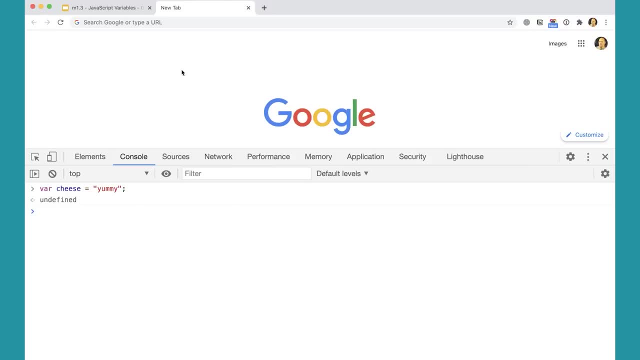 So don't worry about the fact that it says undefined here. Now that I've defined this variable, if I type cheese, you'll see that I get yummy. That comes back. That's the return value for that variable, for that variable name. 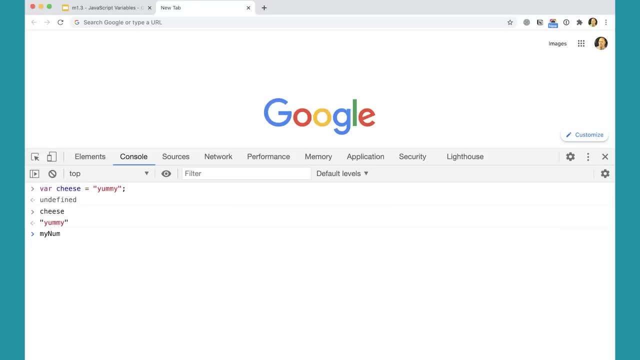 I'm going to make a new variable, myNum, and assign it a value of 5.. And I get a 5 back That returns the value of 5.. So I could make another variable. When I created myNum, you'll notice. 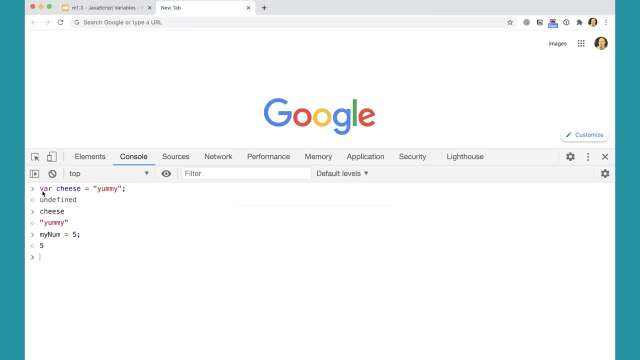 I forgot to use the var keyword, And that's fine. JavaScript will adjust for that in this case, And we'll talk later about what happens when you don't use the var keyword, But in this case it's fine. It actually created a variable called myNum. 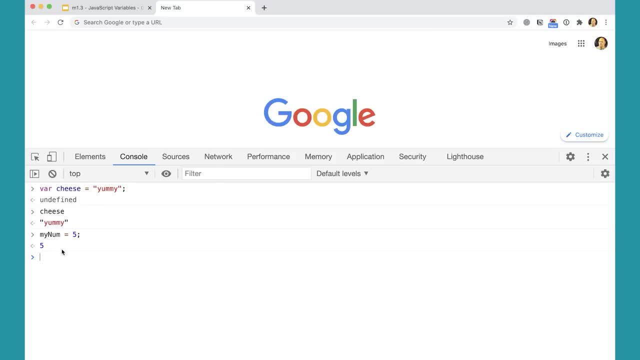 and assigned it 5.. But it would be better to use the var keyword var myOtherNum. So if I do myNum, you'll see I'll still get 5.. If I do myOtherNum, and you'll notice that in Chrome. 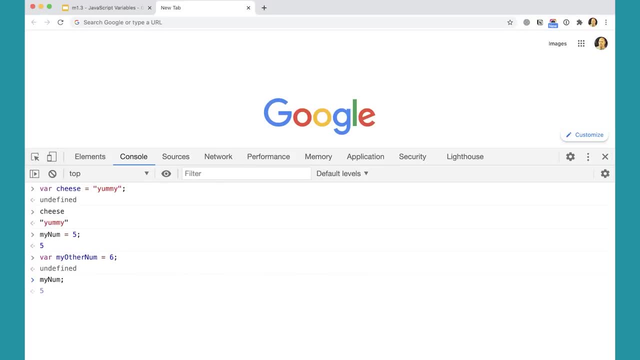 it's predicting what I'm going to type, And if I press Tab on the keyboard I don't even have to type that whole thing. So I'm going to use myNum and I'm going to use myOtherNum, And I'm going to use myNum and I'm going to use myOtherNum. 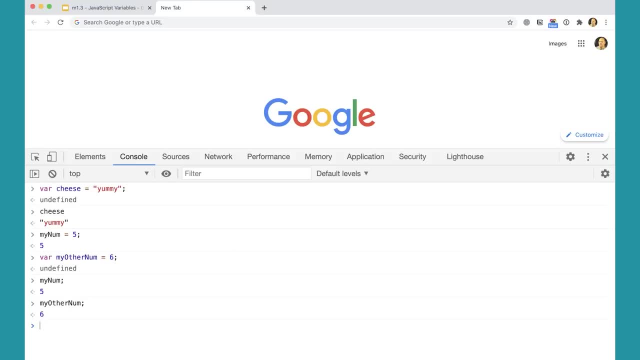 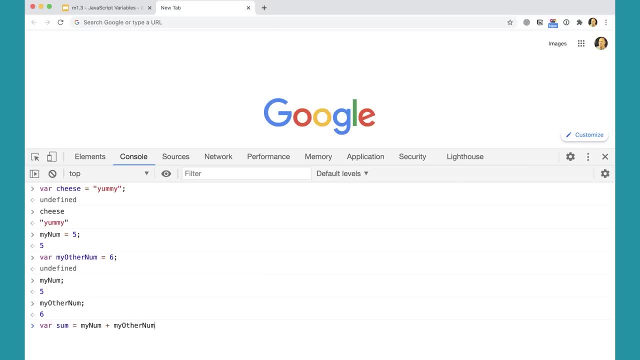 I can even pick it from the list using my keyboard here, So I don't even have to type it. Now, if I do sum, You'll notice I get an 11, because it's doing basic arithmetic. I can also use a method called consolelog. 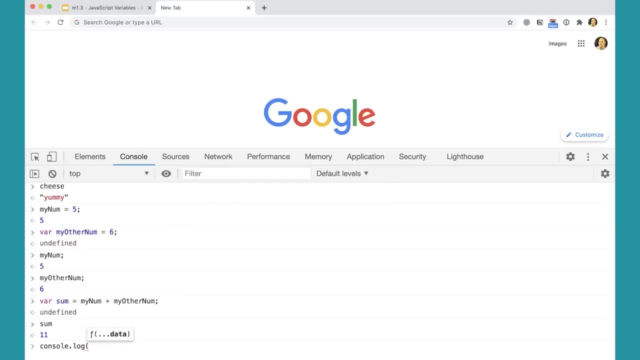 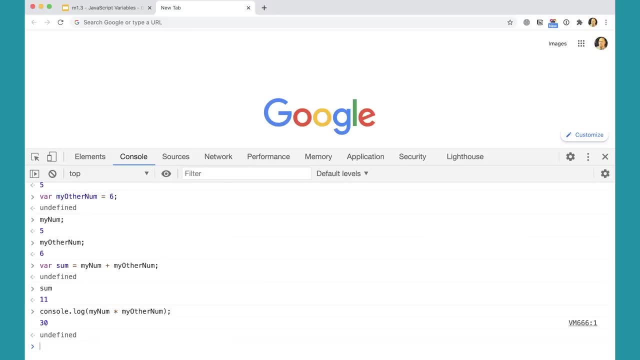 councline And you'll notice that I get 30, because it's taken five and multiplied it by six. Now we're in the console, So we don't have to use the consolelog statement here, the consolelog method, Because I can just do myNum times myOtherNum. 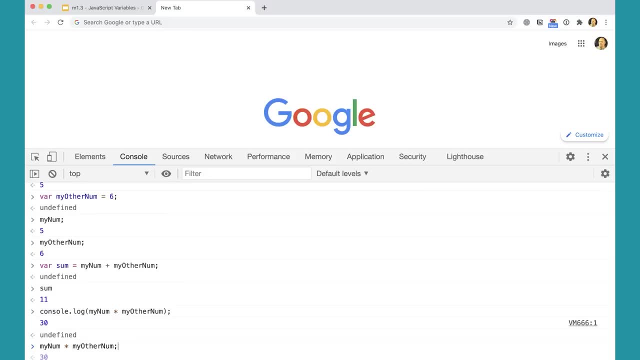 and you'll see I still get 30. but I'm showing you the consolelog method because when we start working with files we'll use this method a lot to send things to this console. While I'm in the console, I don't actually need to use it. 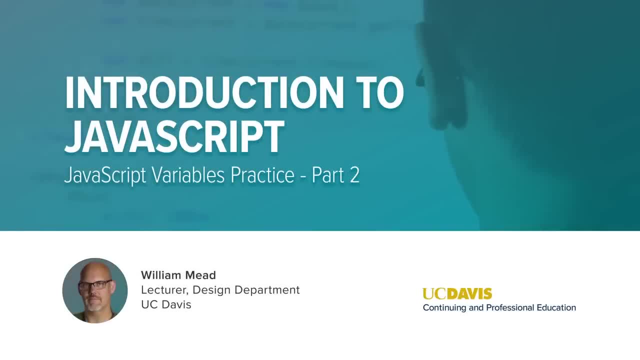 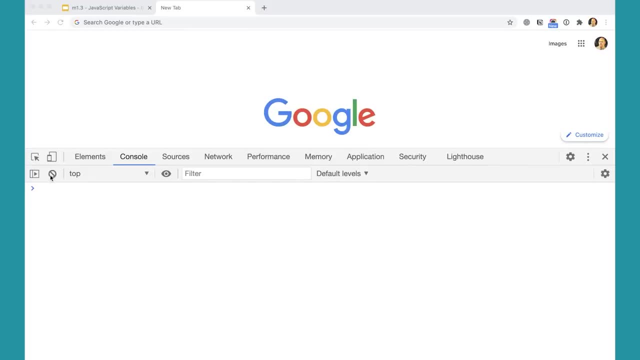 Here you can see I've cleared out the console by clicking this clear thing here. That won't actually forget any of the code that you put. If you do want to actually forget the variables, you can click the refresh button up here and that will actually forget it. but now I'm getting the 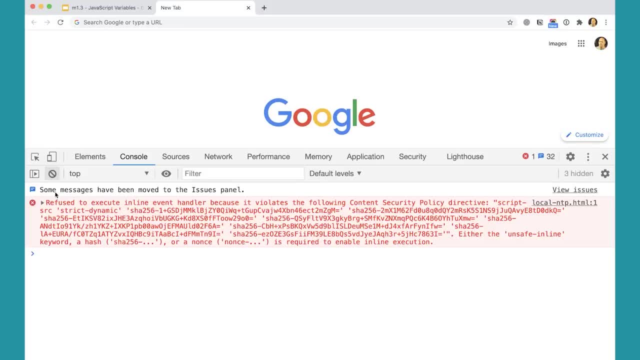 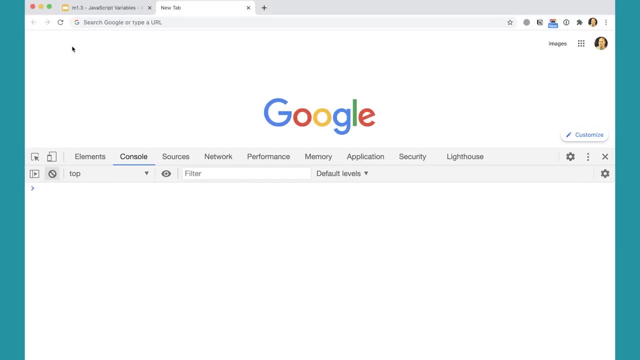 error that came back just with the Google page, but I can clear that here So I can actually create variables fresh that way. So use this refresh button if you really want to clear out what your code remembers. So now, if I were to type cheese, it'll tell me that. 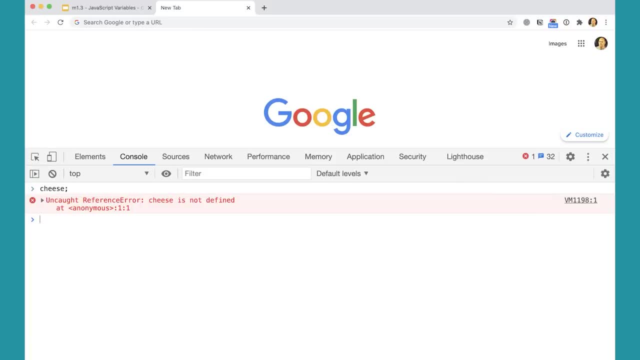 it doesn't have cheese as defined anymore because I refreshed the page. But let's do this. I'm going to make a variable, var, not num. I'm going to assign it a value of five, but I'm putting it in quotes because it's not really a number, It's a string with the number in it, And I could make: 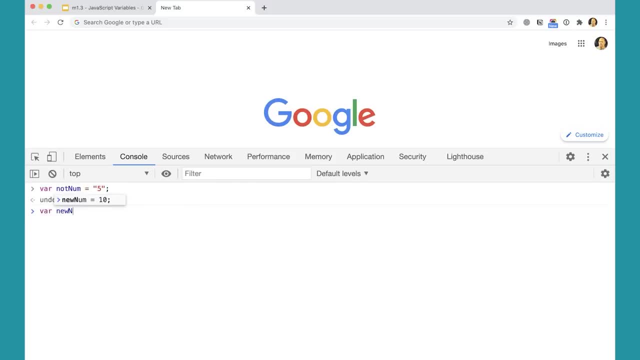 another variable, var. new num. I'm going to assign it a value of ten, So that's it. That's actually a number. Now watch this: If I do new num plus, not num, it gives me a 105 inside quotes. Now JavaScript is loosely typed, You do not have to specify. 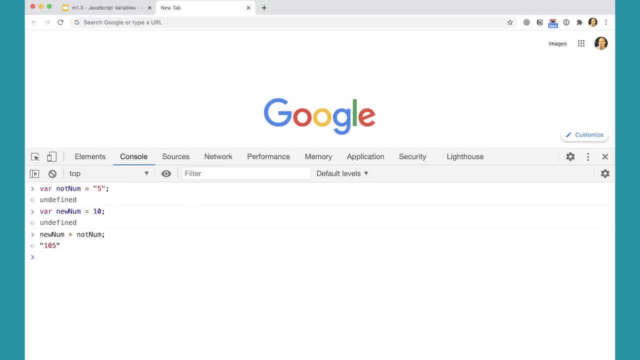 what type of data a variable is going to hold when you create the variable. And a lot of people don't like that about JavaScript, And way back in the day when they were working on ECMAScript 4- you'll remember that version was never released- They were thinking seriously about switching. 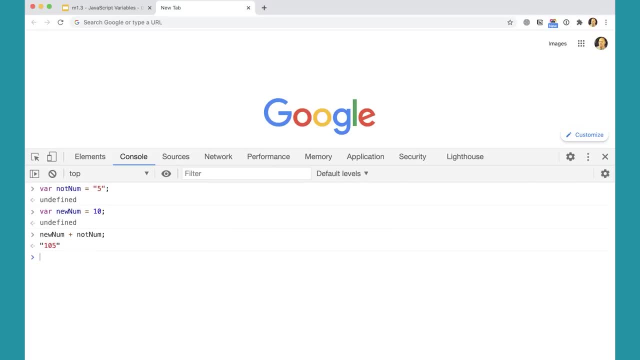 to being a more strongly typed language, like other languages, where you have to declare what type of data a particular variable will hold when you create the variable. But in JavaScript you don't have to do that, And Douglas Crockford, who we mentioned earlier, made a strong argument that 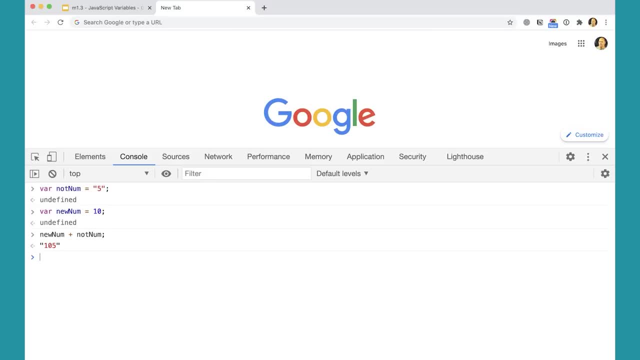 the loosely typed nature of JavaScript is actually very expressive and very powerful in its own way If you know how to type JavaScript. you can type JavaScript in a very expressive way If you don't know how to use it properly, But it can lead to confusion, And here's a good example of that. 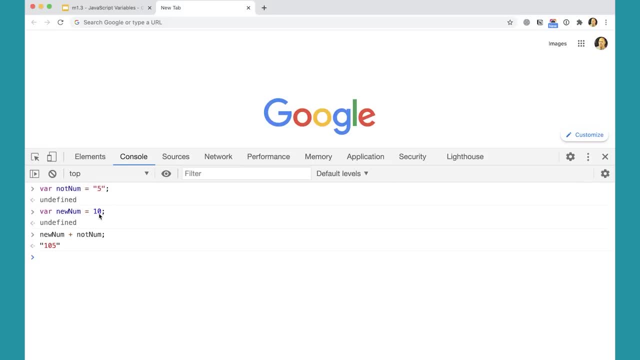 Where you might get something that we don't expect. Perhaps we expected to add 10 to 5 and get 15. But instead we got 105 in a string. So that's kind of an important distinction and something important to understand about the way JavaScript works. Another thing to note is that 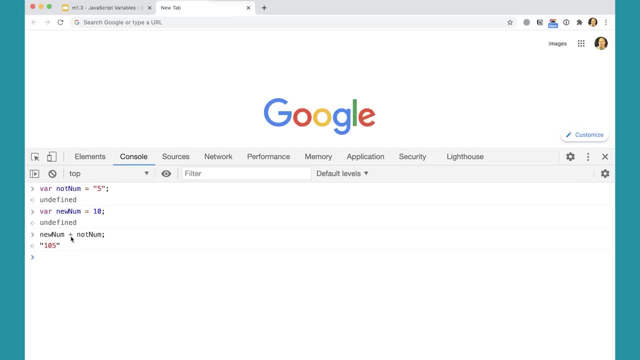 the plus operator in JavaScript does double duty. It will add numbers together. So we could make another variable, var newNum2 and assign it a value of 6. And then I could do newNum plus newNum And it will give me 16. So it will add numbers together, But it will also concatenate strings. 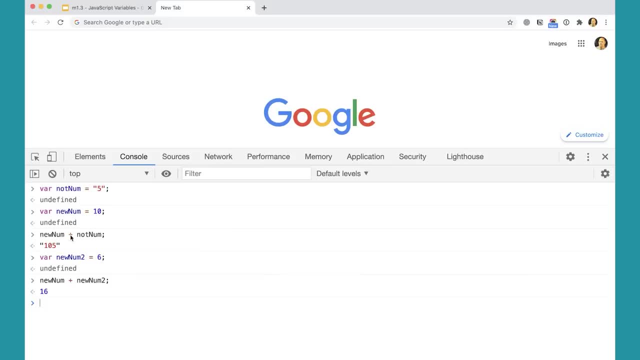 So here we were seeing the plus sign actually doing some concatenating, because one of those elements was a string, So it concatenated it together And I got 105.. And down here when we use the plus sign, it's actually adding: This is a problem in JavaScript And they've done some things in the language. 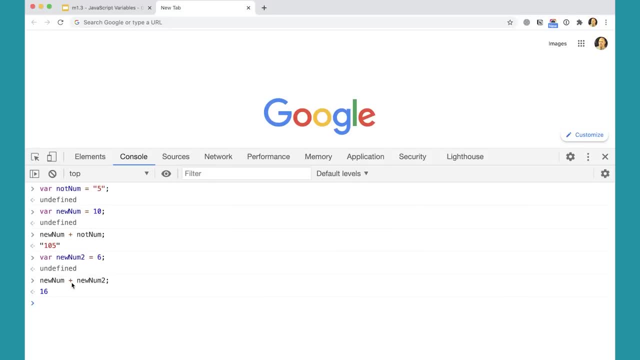 to help mitigate the fact that the plus sign does both things, And we'll look at what we can do to deal with that. We'll look at some better ways of putting strings together other than using the plus sign. But these features of JavaScript that were built in from the beginning persist to this day. 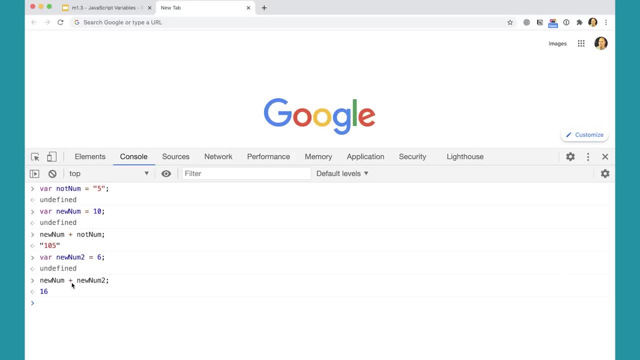 And the plus sign still does two things: It concatenates and it adds. So here we're seeing already very much at the beginning of the course, this plus sign, things about JavaScript that are a little bit different. We're seeing that it is a loosely typed language. 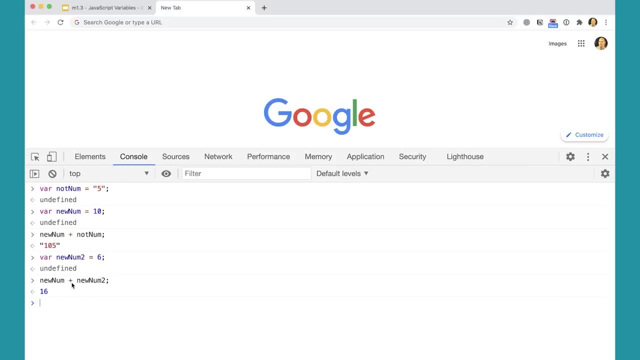 and that's unusual. We're also seeing that the plus sign does double duty, and that's not only unusual but a little bit problematic. And so already you're learning a little bit about why we use JavaScript in certain ways or why we type in certain ways. 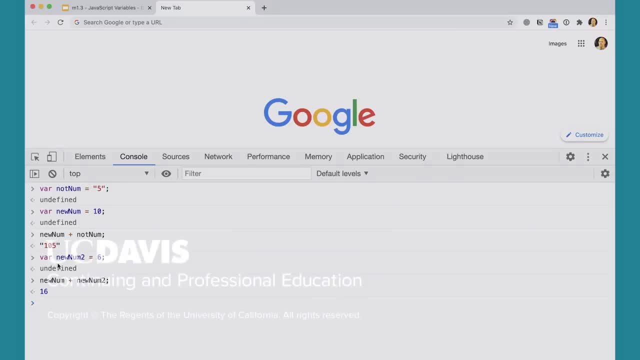 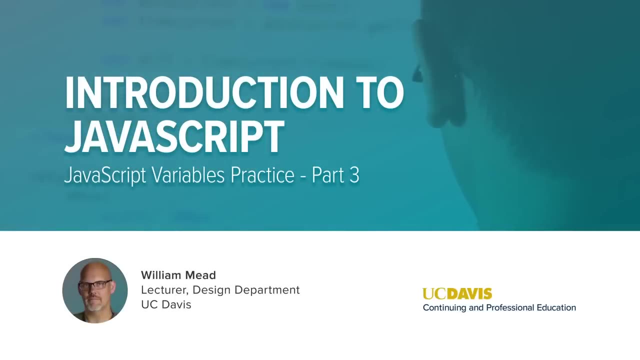 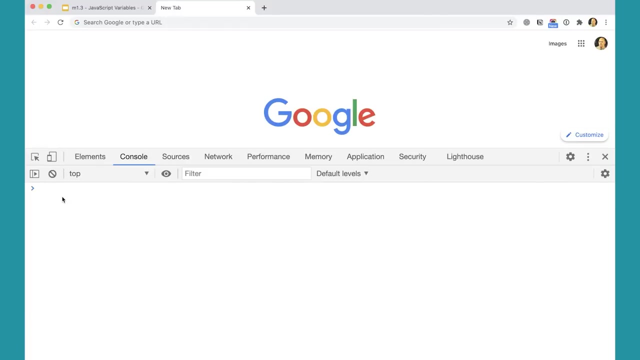 And we'll get into more detail about that as we go along. I'm going to clear out my console here- That's the clear button there- And then I'm going to create a new variable: var myNum equals 10.. I'm sure we'll put that in there. 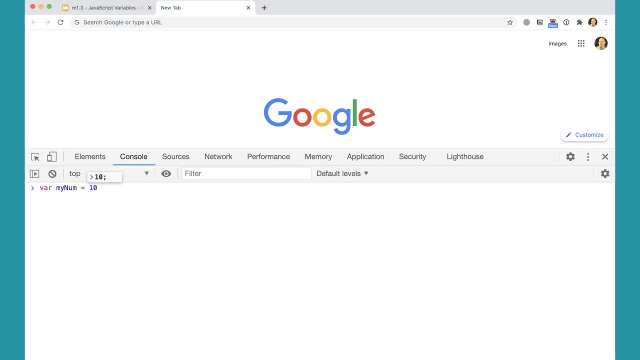 And then I'm going to make another variable: var myNum equals 10.. I'm sure we'll put that in there. var myNum as string. I'm going to make a variable there and I'll call it five, But that variable again is a string. 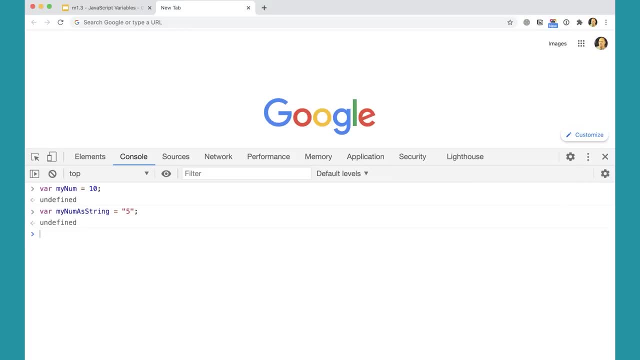 Now it's important to note that even though JavaScript is loosely typed, it doesn't mean that variables don't have a type. So if I do type of, which is a method that allows me to pass in a variable like myNum, it'll tell me that it is in fact a number. 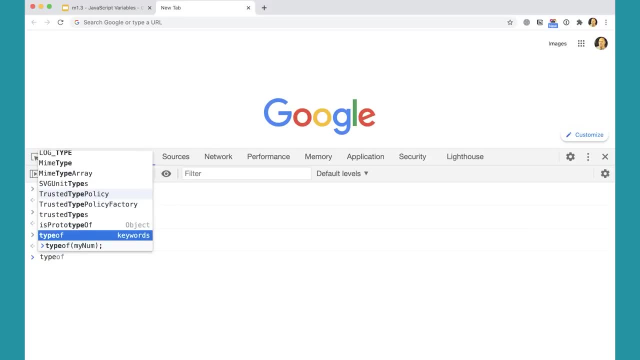 Whereas if I do type of myNum is string, I can actually pick it from the list here, so I don't have to type the whole thing. It'll tell me that it's a string. It'll tell me that it's a string. 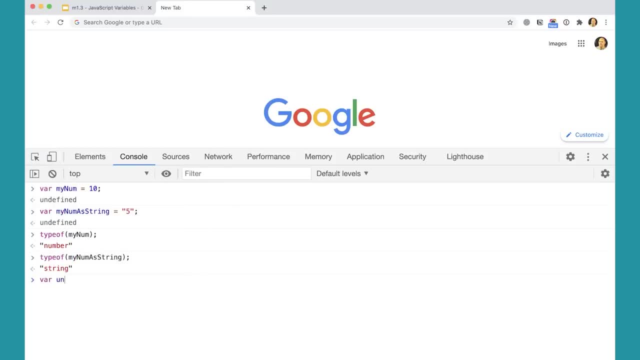 If I make a variable, var undefined variable and leave it empty, so there's nothing in here, I could do type of undefined variable to get my variable here and you'll see that I get undefined. or I could do var nothing at all and assign it no. 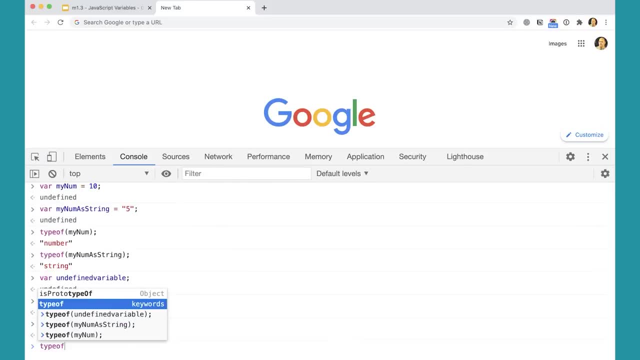 and I could do type of nothing at all and I get object. So that's kind of interesting. So these are some of the first things that I've done. So these are all very different variables with different values, And that's an important thing to understand. 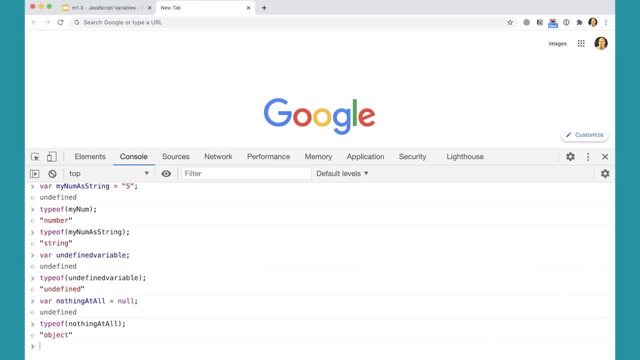 about JavaScript, But they do have type associated with them. Let's try one more. I'm gonna make another variable, var, empty string, And I'm gonna assign it a couple of quotes. And if I do type of empty string, you'll see, even though there's nothing in there. 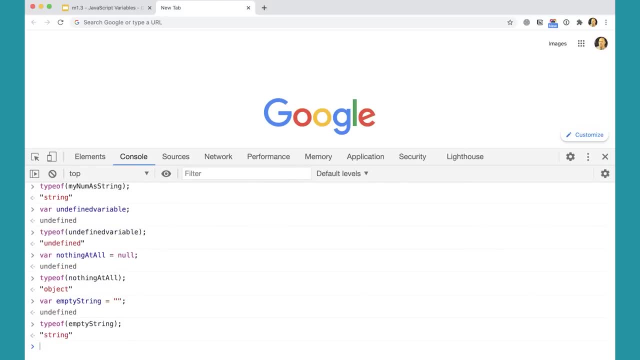 there's nothing really assigned to this variable. The fact that I put a pair of quotes there means that it is in fact the string. It's also kind of important to note that I could use single quotes or double quotes in JavaScript. They do the same thing. 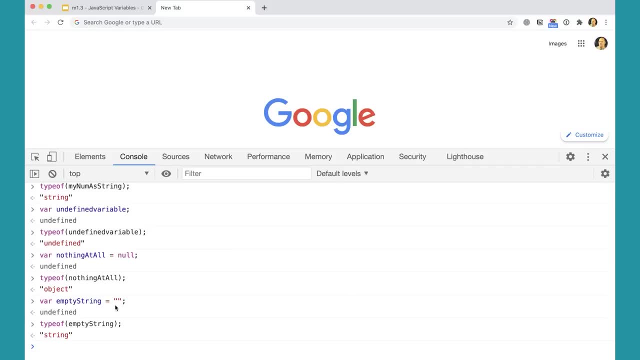 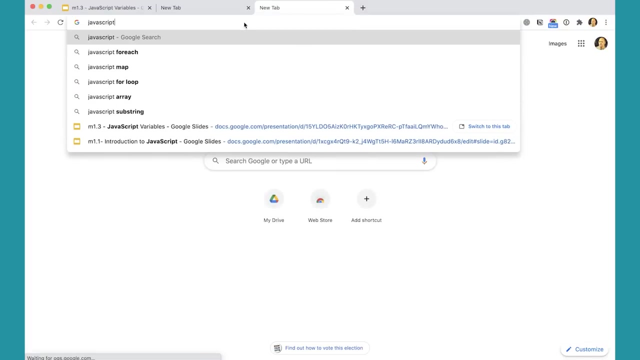 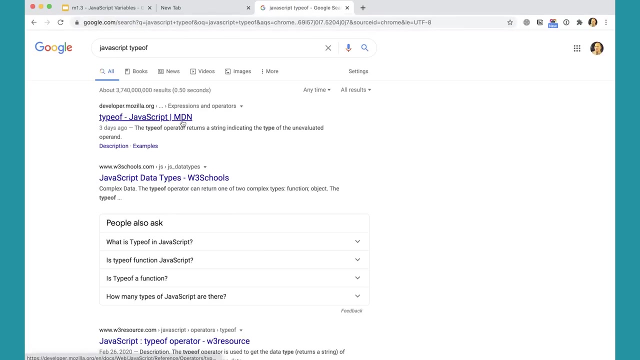 So it doesn't really matter if you use single quotes or double quotes at all. Now, if you wanna find out more about the type of method, you could come over here and just Google JavaScript type of, And the MDN will come up very quickly, if not the first. 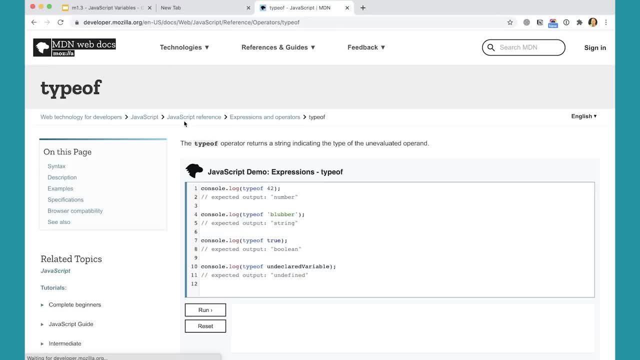 Sometimes you'll get W3 schools. The MDN, which is the Mozilla Developer Network, is the definitive resource for web technology, such as HTML and CSS, And we'll give you a lot of information about different methods and different things you can use. 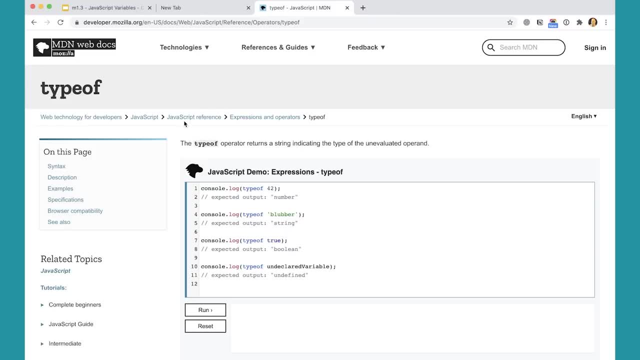 And we'll be referring a lot to the MDN throughout this course, Sometimes the W3 schools website as well. But the MDN really is sort of the definitive resource, but it can be a little bit confusing at first. So sometimes the W3 schools website. 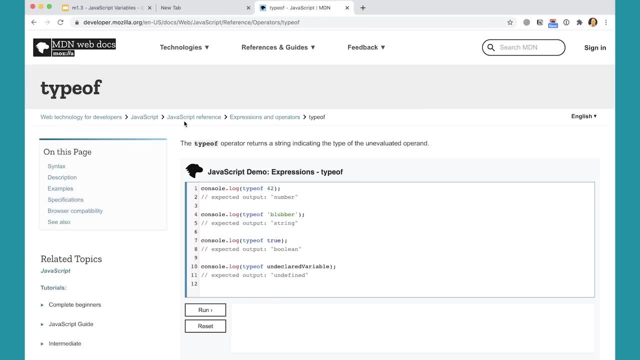 is a little bit easier to understand, But the MDN is very thorough. Okay, so that gives us kind of a very basic start at creating some variables that can hold different pieces of data. And at this point you're probably wondering: yeah, so what? 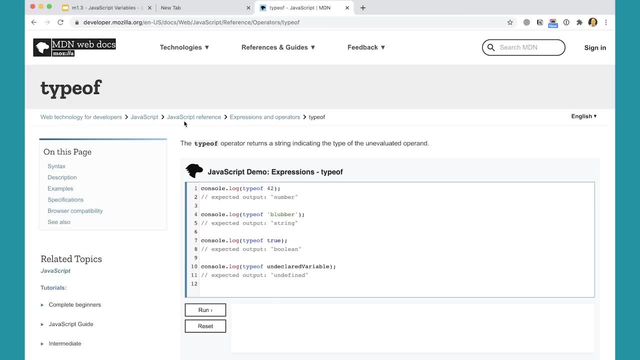 But remember that as we're learning a language right now, we're just learning the alphabet, And the letters by themselves don't really do all that much. It's not until you start putting them together to form words that can start to have meaning. 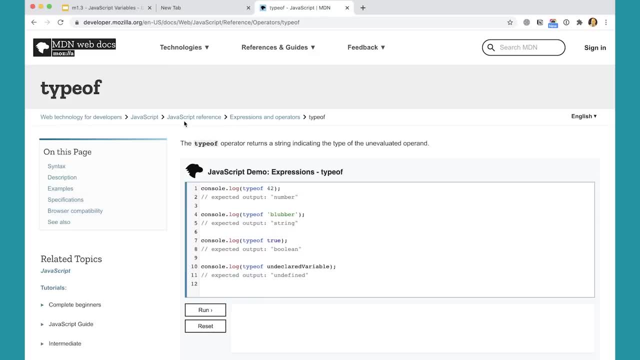 So we'll be working on some more of these very basic elements of JavaScript, But then, pretty quickly, we're gonna be getting into more interesting aspects of the language and you'll be creating more interesting little programs that will actually do things on web pages and on websites. 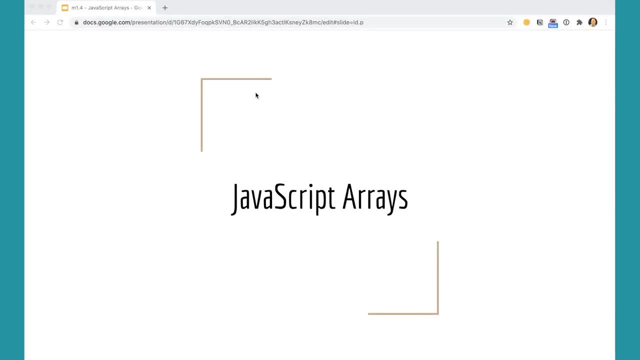 So let's get started. JavaScript arrays. An array is really just a container with subcontainers, And it's the next piece of the puzzle that we need to talk about in terms of JavaScript. We talked about variables, and an array is just another type of variable. 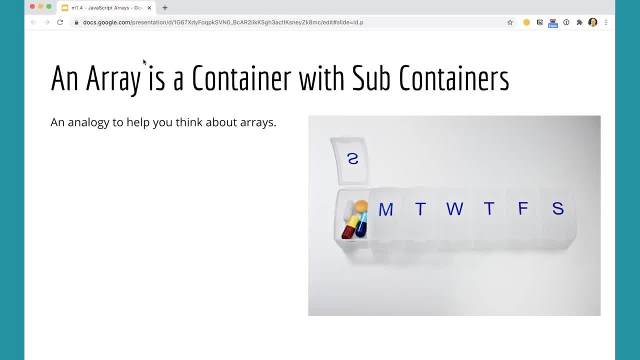 But instead of holding one piece of data, it can hold multiple pieces of data. Think of it like a pillbox, right? Perhaps you or a friend or a relative has to take medications each day, And perhaps they have a box that looks like the image here. 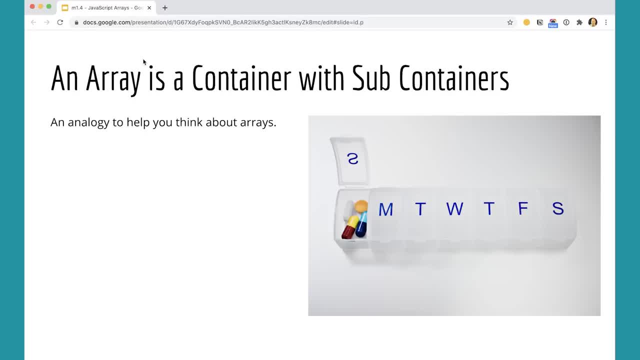 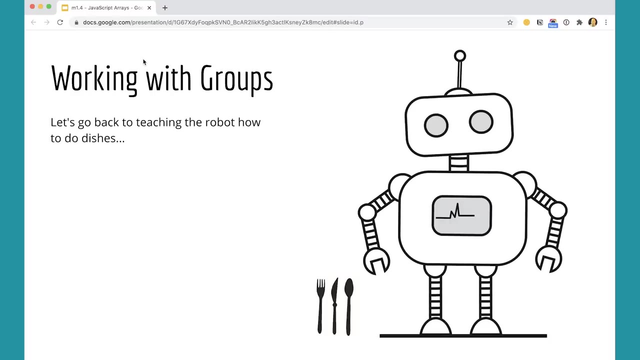 on your screen where you have different containers that are gonna hold different things, different pills for the week, And frequently in JavaScript we have to deal with groups of things. And if we go back to our robot analogy, if our robot, if we're teaching our robot how to wash the dishes, 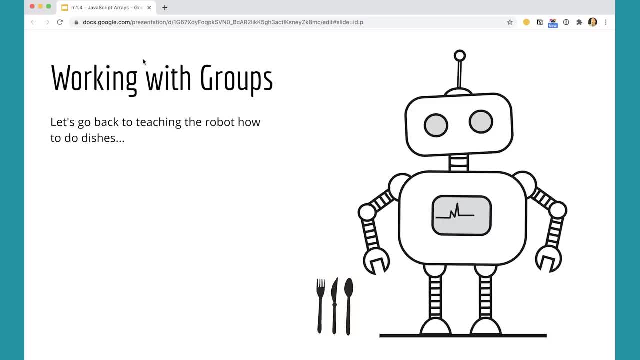 perhaps glasses need to be handled in a certain way, or perhaps plates need to be handled in a certain way. And then, when it comes to working with the silverware- you know we've got, the silverware needs to be handled in a certain kind of way. 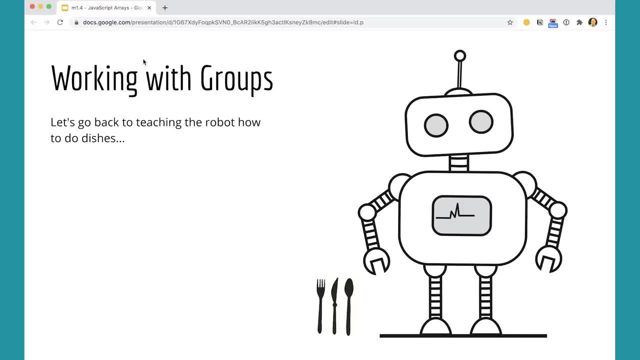 but then we've got a subgroup of spoons and knives and forks and maybe other pieces of silverware. So that's a group within a group, And arrays are the analogy that works best, for that is thinking about groups of things with arrays. 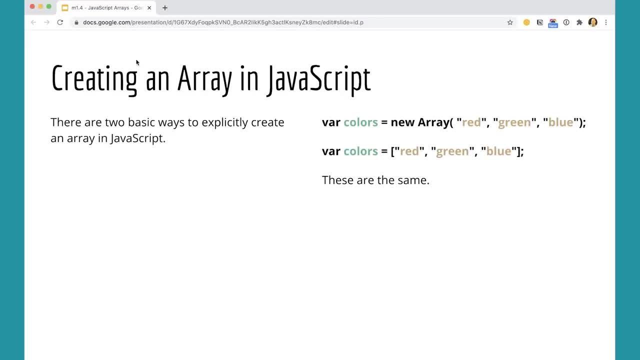 So let's take a look at what that looks like. So in JavaScript, we can create a new array in a couple of different ways. We can use the new keyword with array and parentheses, as shown here, or we can use we can create it more explicitly using the square brackets. 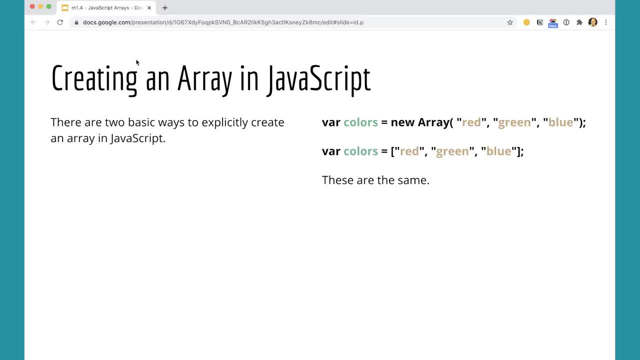 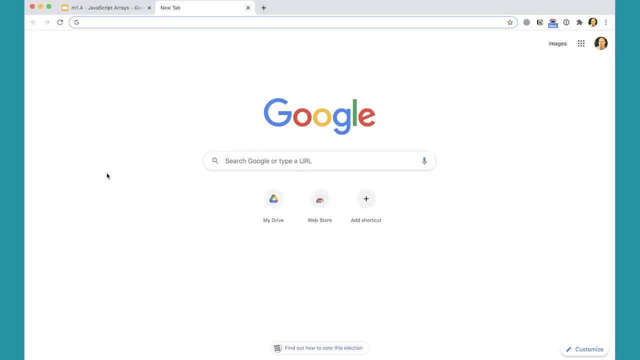 as shown below On the right here. So let's actually do this over in the console. So I think it's helpful to actually see us create these, create these elements. So I'm going to come over here and make a new tab and choose inspect. right click and choose inspect. 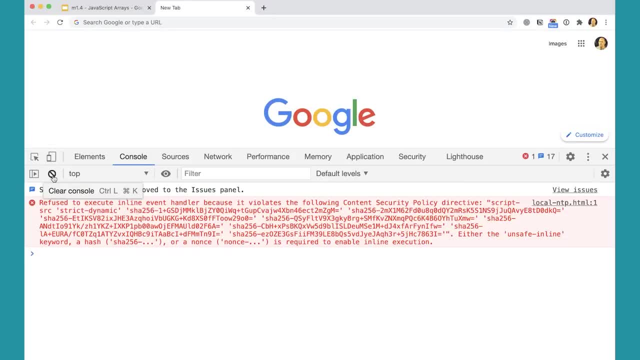 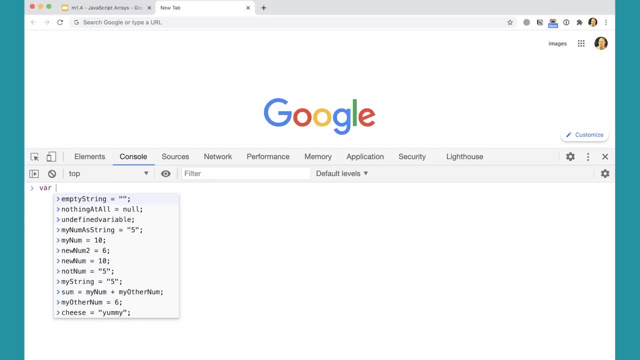 And then click on the console here clear out this error. I don't need that stuff. but then I'm going to make an array var. I'm going to call it colors1.. equals new array and then in here in quotes I'm going to put some colors. 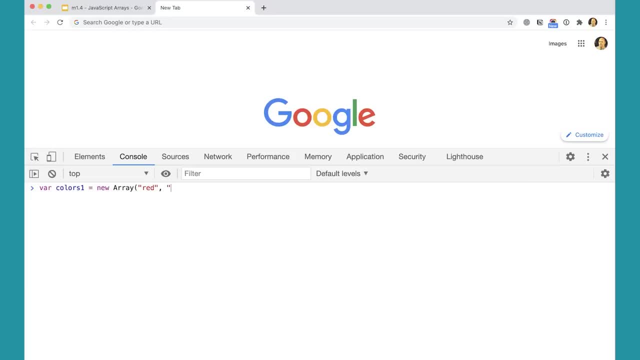 red comma, green comma, blue. Now I've created this main dash here working with a function called tag command, So let's see additional names for this. Here we go. Now I've created that array and I can access those colors by typing colors: one square bracket, zero and square bracket, and that will get me the first color in that array. 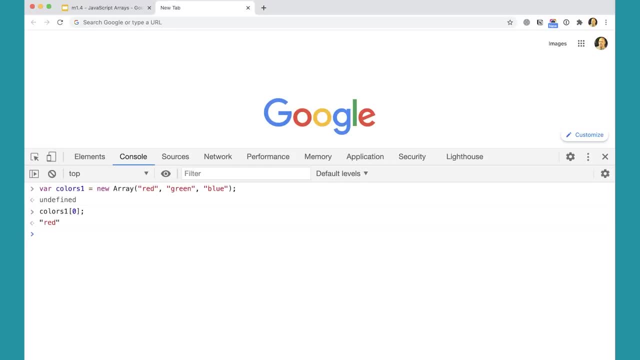 That'll get me the red, Or I could make an array more explicitly, and this is the more common way that you'll see it done is: bar colors, two equals square bracket and then quote yellow, quote orange Or quote purple square bracket, semicolon. 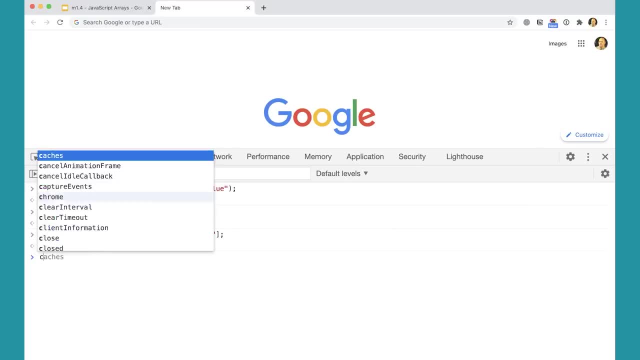 So now I've created a second array and I can do colors two, square bracket two And that will get me the third element in the array. Now square bracket two gets me the third element. That's weird: Arrays are zero-indexed. 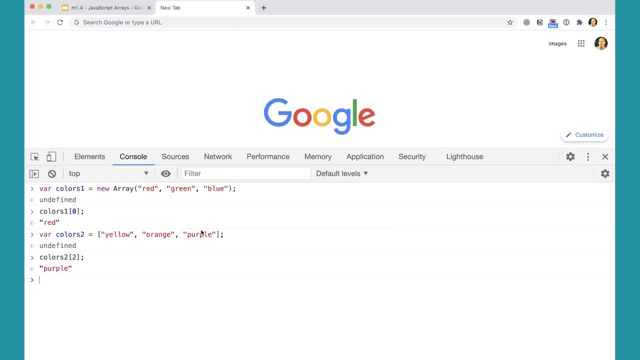 So this is element zero, this is element one and this is element two. This is element zero, element one, element two. But the length of the array is three Colors, two dot length. That will give me a three Because there are three elements in the array, it's just they're numbered zero, one and two. 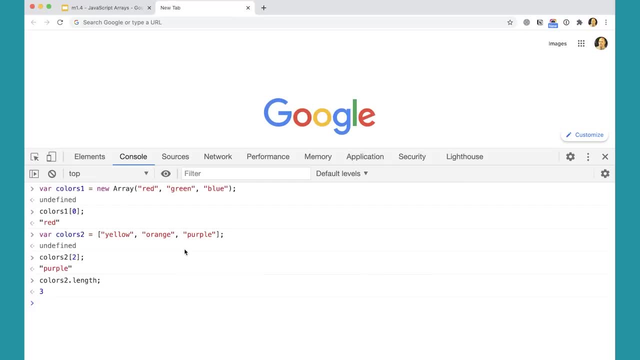 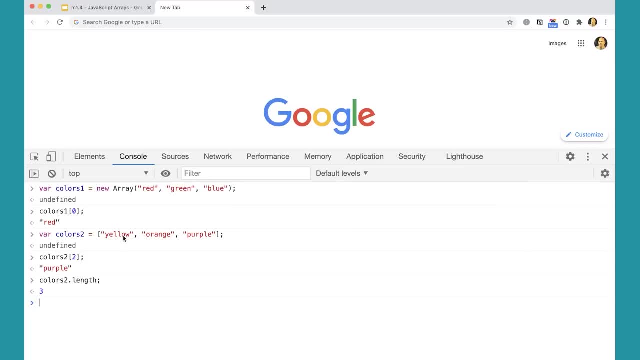 where, when you have an array, the first element is element zero, and then a one and then a two. Normally we start counting with one first, one, two, three, But in programming we frequently start counting with zero first, zero one, two. 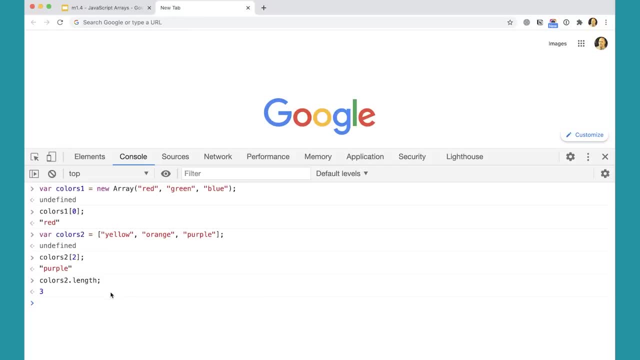 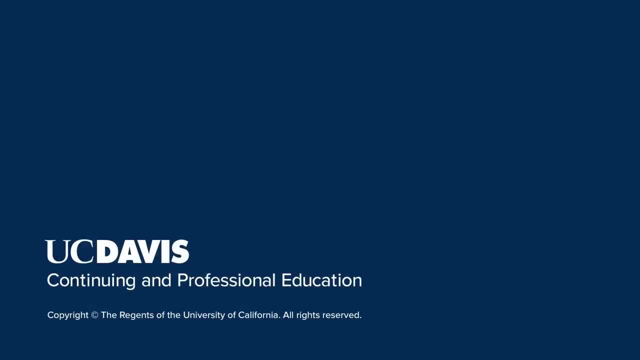 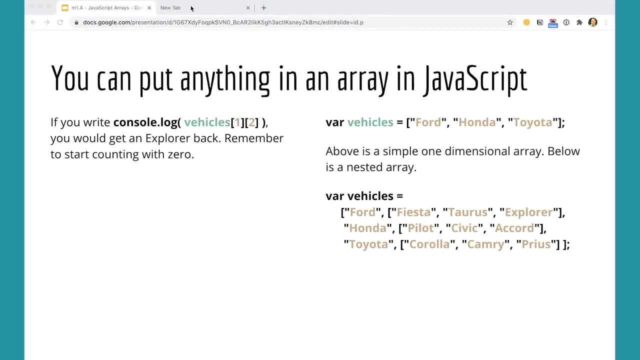 But the length of the array is three, three. So that's an important distinction and something to be aware of. Unlike a pillbox, which really can't hold much more than just pills, you can put anything into an array. in JavaScript You can even put an array in an array, So you can think about a pillbox with. 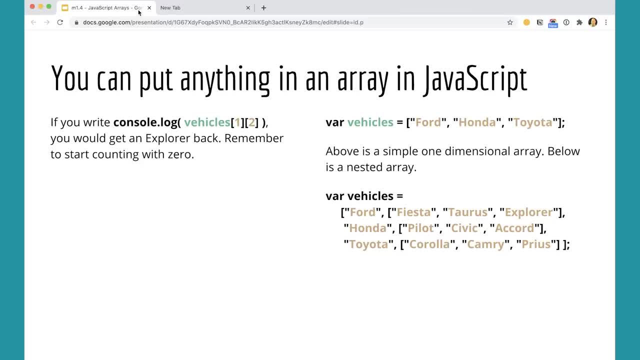 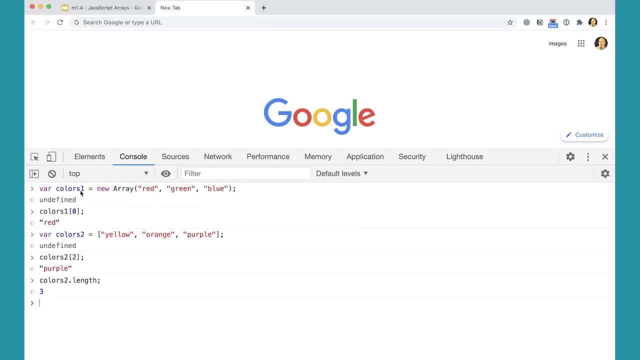 a subcontainer with even smaller divisions in it. So let's take a look at what that looks like. I'm going to switch back over to my tab here and I'm going to clear out this tab by clicking the clear button there And I'm just going to paste this in. but 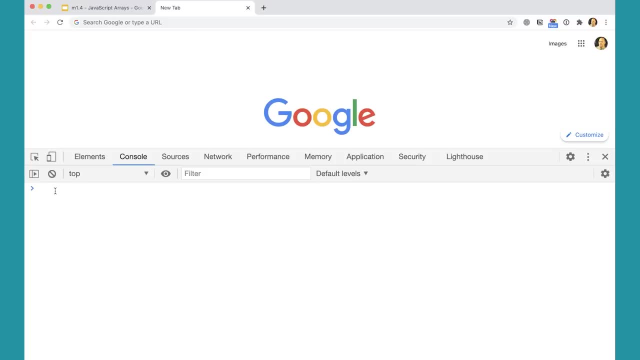 you might want to type it. It's a little bit hard to type and get right, but it's worth trying. if you can, I'm going to paste this vehicles array in here And now, if I do. if I want to access an element from this array, I could do vehicles. 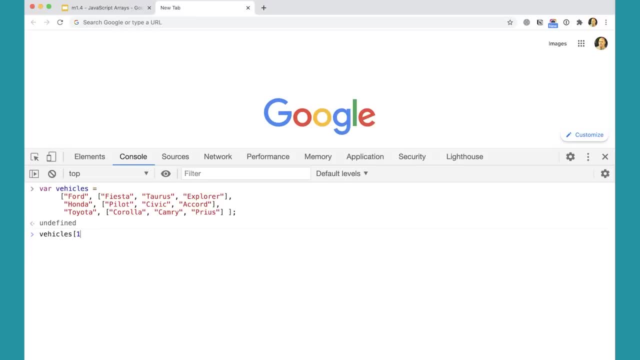 square bracket one That's going to go and get the line that starts with which element. There we go, And then so it's going to get me this, because this is zero, and then this is one, All right, so that's going to get me that into that subarray. 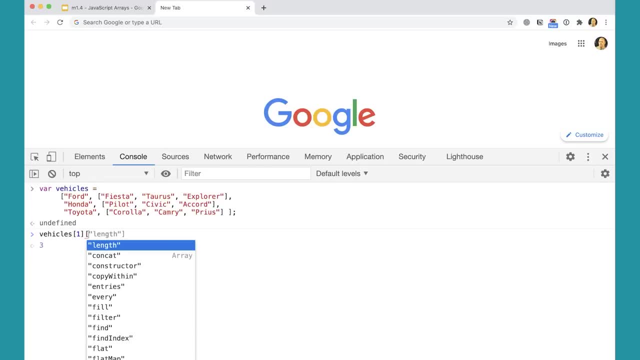 You can see it sort of showing up down there And then if I do square bracket two, that's going to get me the explorer element in that subarray. So you can do things like that with arrays. That's kind of complicated and you're not probably going to be doing. 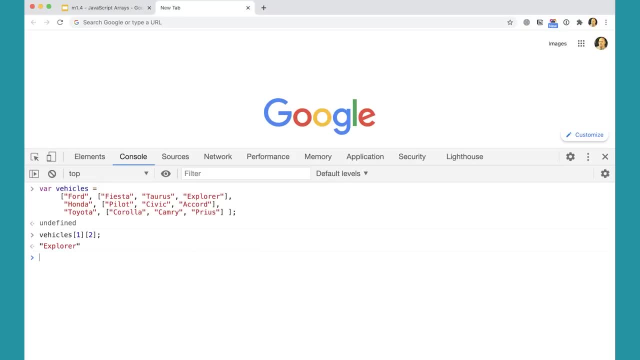 arrays inside of arrays to start off with, But it's an important thing to understand About arrays. they're very flexible tools that you can use to hold groups of data, and that's very useful. Another thing that's interesting is that a regular variable holding a string can be treated like an. 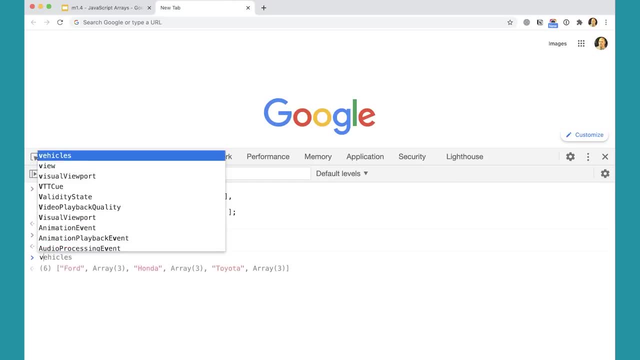 array in JavaScript. So if I make a variable var, joke equals the chicken crossed the road. Now I've got a variable called joke but I can actually treat it like an array. I could do joke square bracket four And that's going to get me the c in chicken. 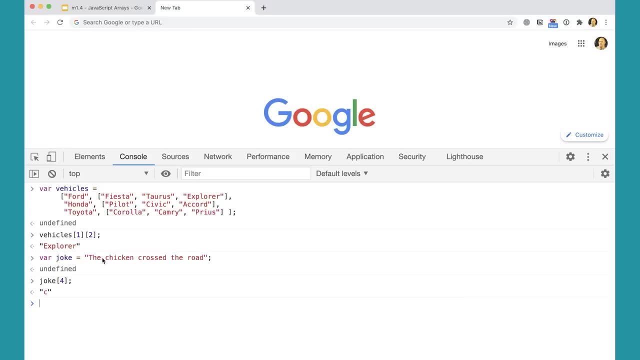 Because 0-1-2-3-4. is going to get me that c in chicken, Or I could do joke dot length. It'll tell me that there are 28 characters in that string. So that's kind of an interesting thing to understand about arrays as well. 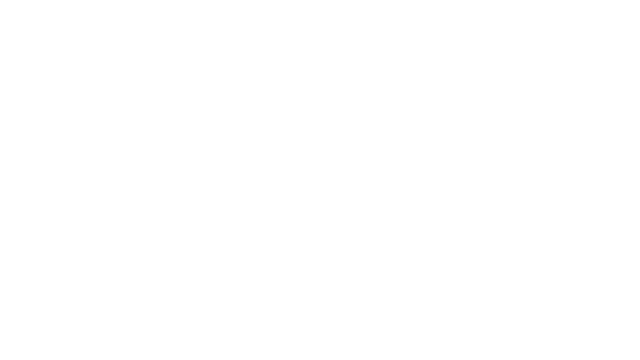 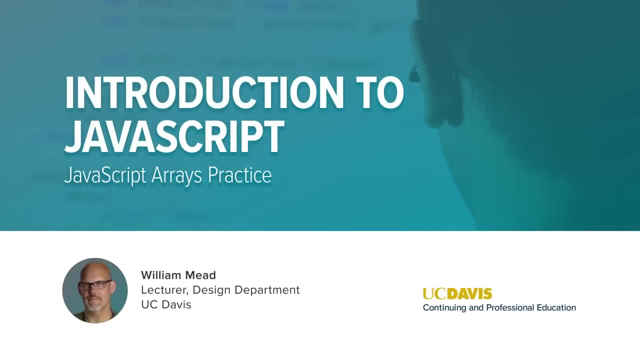 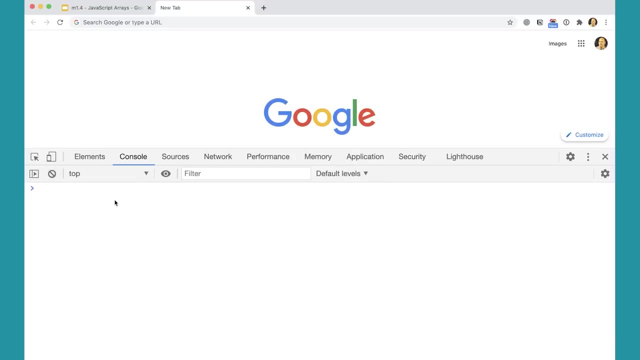 It's kind of a loop to type and change the orbit of the string. Let's do a little bit of practice with arrays So I can make a new variable, var animals, and assign it an array- cat, dog, chicken- and all of those animals will be in the array. 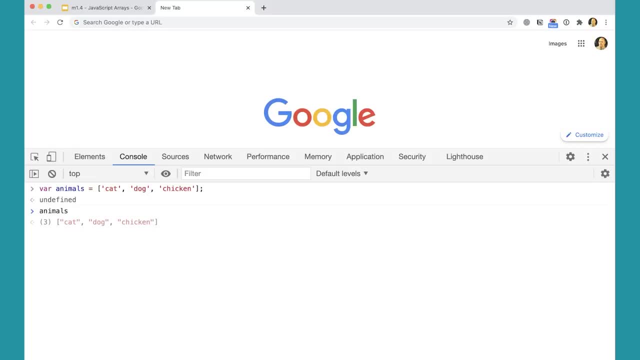 So if I just do animals, you'll see that I get back an array with three elements: cat, dog and chicken. Now arrays come with certain array methods that you can do to arrays specifically. So if I do animalspush Now, there are four elements in the animals array. 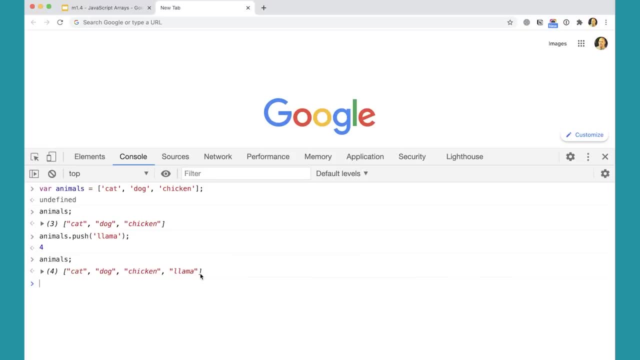 The cat, the dog, the chicken and the llama are all in the array. Remember we can use the console log method. We don't really need to here in the console, but we will when we go to using files shortly. So it's worth remembering that we can do consolelog. 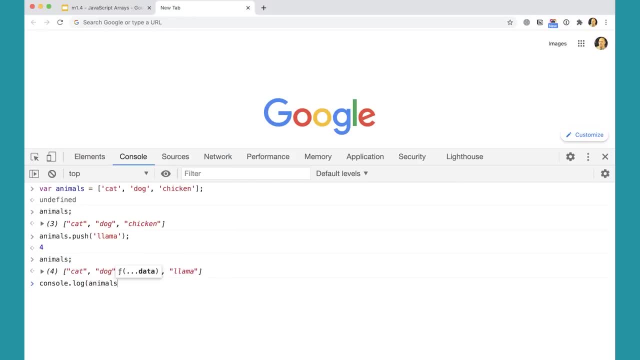 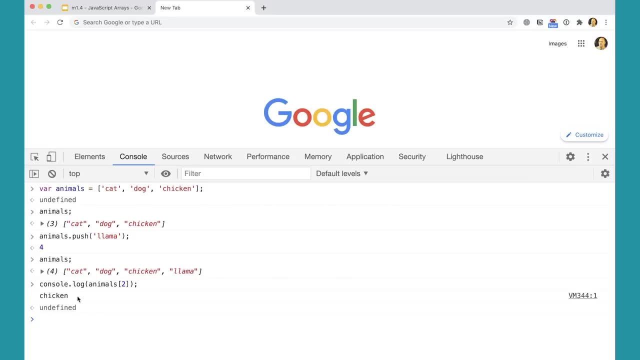 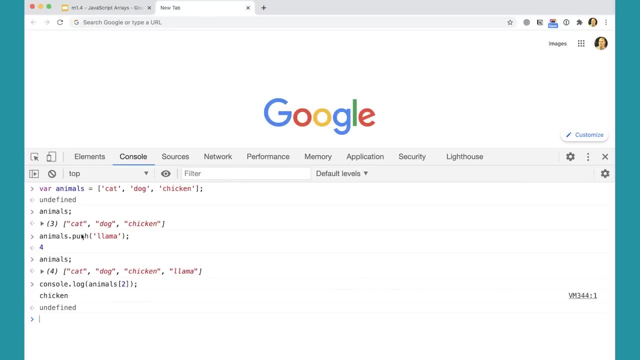 and it's worth remembering that you can do that. Now, what if I wanted to remove an element from the array? Well, we could do animalssplice And that will take the dog out of the array. So now, if I do animals, you can see it's got the cat, the chicken and the llama, but not the dog. 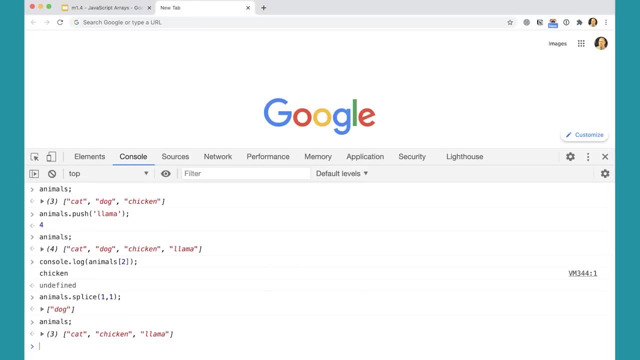 And I could do push and push the dog back into the array. Let's do that Animalspushdog, And now the dog is back in the array. Another array method is sort Animalssort And notice now that the order of the animals in the array has changed slightly. 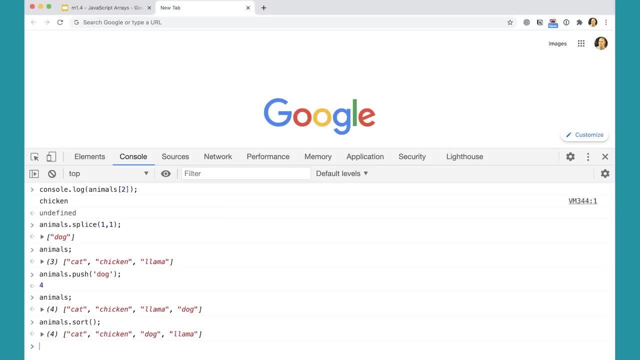 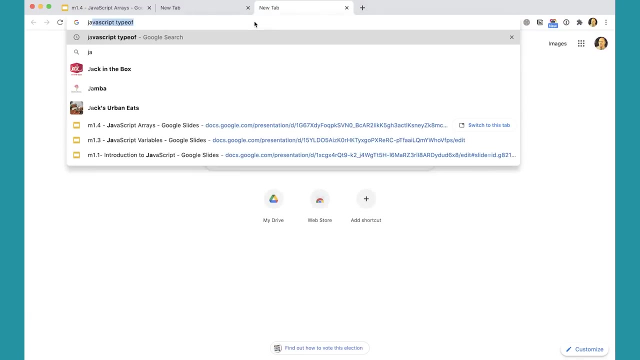 so that the dog is in the third position based on alphabetical order. So there are a lot of array methods that you can use, and a really good place to go look at them would be the W3Schools website or the MDN JavaScript. 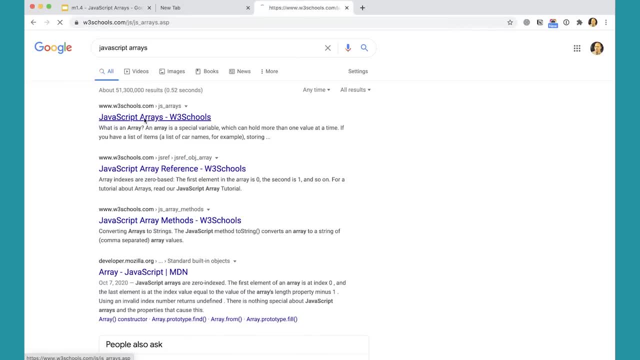 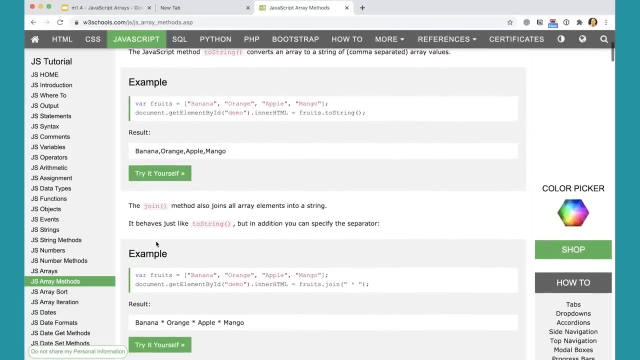 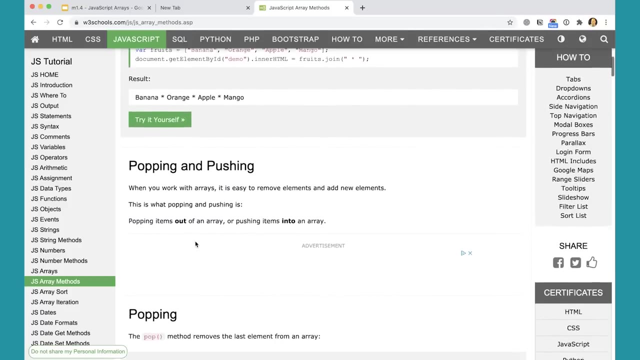 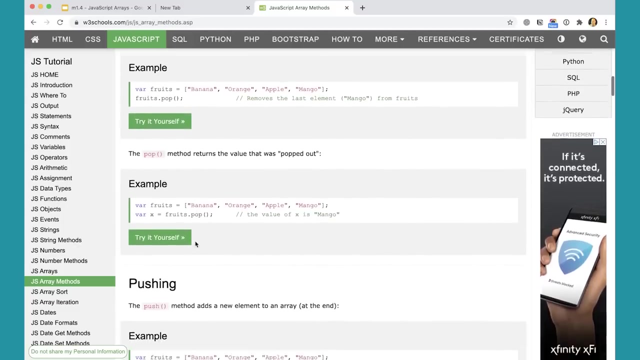 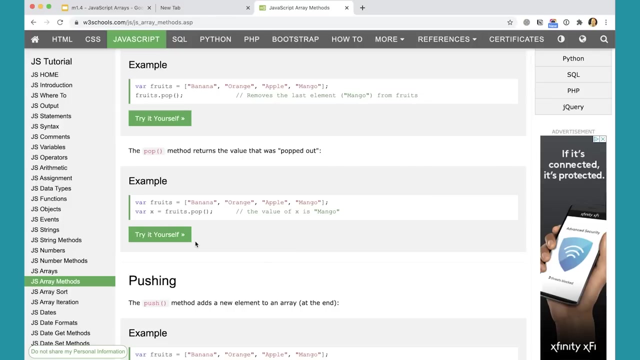 Arrays And here it is here, And then they'll have array methods here And there are all kinds of examples of array methods that you can use. You can join, We can do all kinds. You can do all kinds of things And it's worth exploring some of the different methods and trying them out on your own, with just messing around with arrays and just working in the console and getting used to how this works, because that's a really great way of learning sort of the basics of JavaScript. 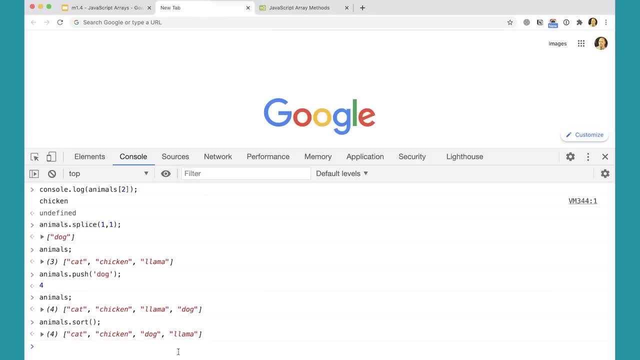 Here's a challenge for you. We have an array for animals here, and we can see that the length of the array is four, But you could also find it And you'll get four. Now what if you didn't know how long the array was? 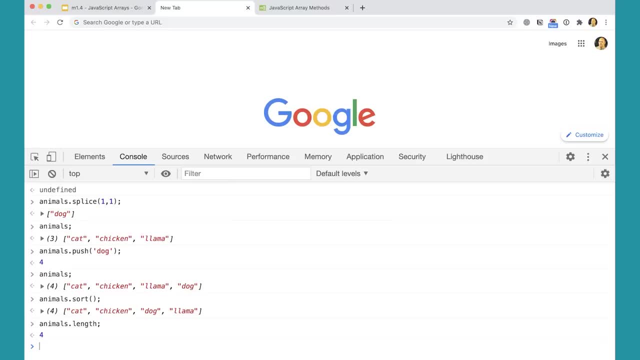 How could you always get the last element in the array? What would be the code that I could type in here that would always give me the final element in the array, no matter how long it is. See if you can figure that out. Pause the video and see if you can figure that out. 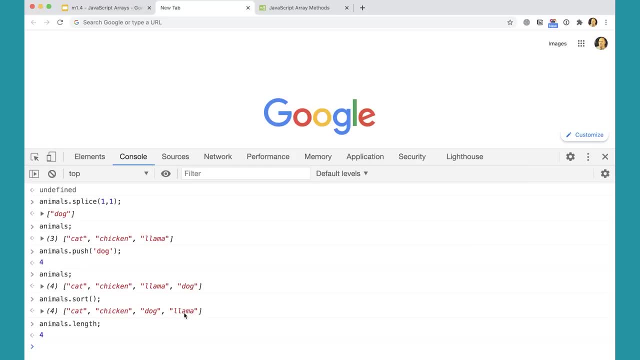 Pause the video and see if you can figure that out. Pause the video and see if you can figure that out, And then you can type in the code that gets that And then, when you're done, you can unpause and I'll show you how I did it. 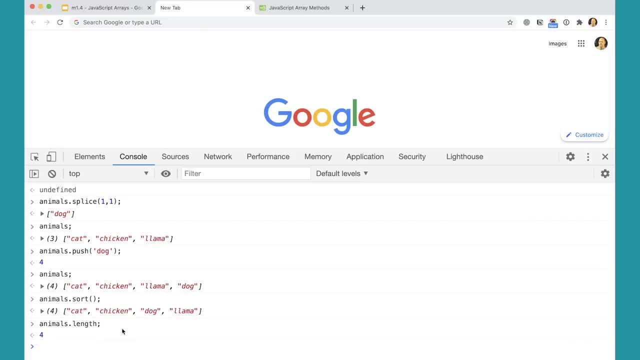 Okay, Hopefully you paused the video and you tried to do that, So here's what I would do. I would do animals and then square bracket And then I want to get the length- animalslength- But I need to subtract one because the length of the array is four. 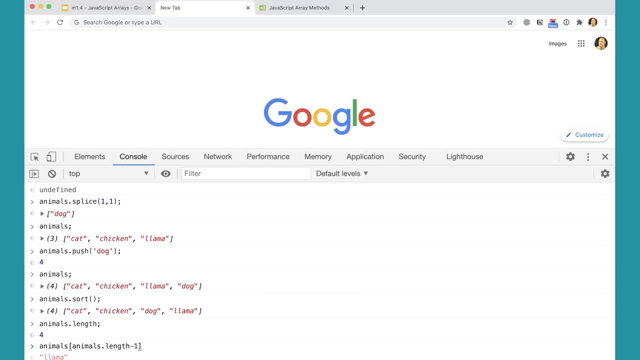 But actually the last element is element number three, And you'll see that that will in fact get me the llama at the very end. So I'm going into my animals array And what I'm passing in is animalslength, which will be a four minus one, which gets me this element here. 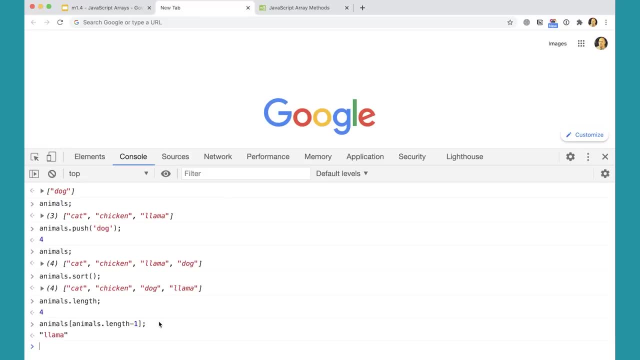 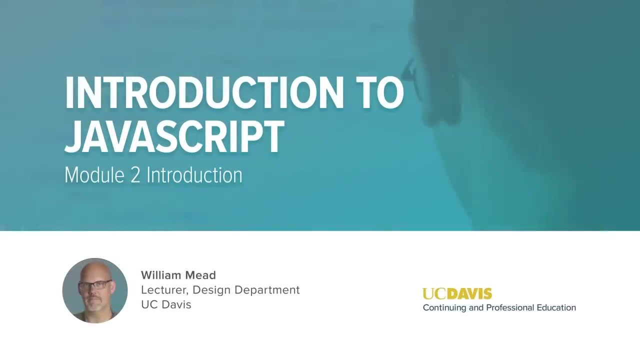 Zero, one, two, three, And that may seem a little counterintuitive to begin with, but you'll get used to working with arrays and with the length of arrays and with different ways of getting elements out of arrays. Welcome to the second module. 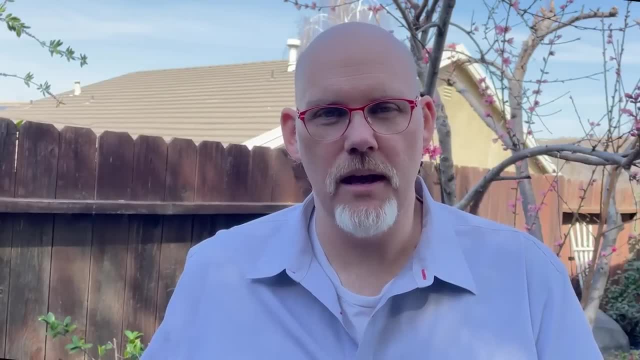 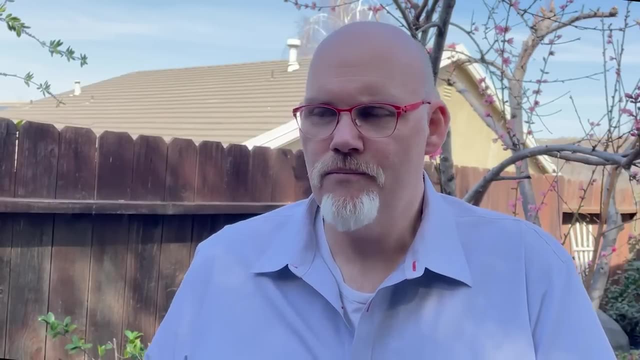 Welcome to the second module. We'll get further into the basics of the JavaScript language. There are certain things that you'll find in many modern programming languages, such as control structures, such as being able to figure out if something is true or how to handle something in a loop, and these kinds of things. 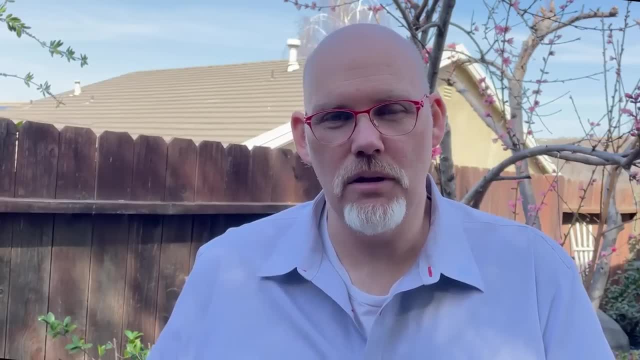 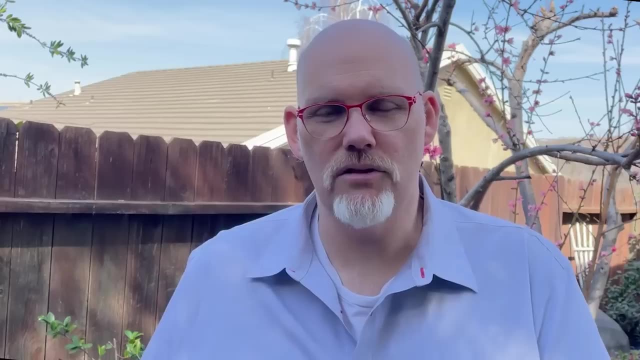 And we'll be doing that sort of work in this second module, And there's a lot of practice and there's a lot of opportunities along the way to really get used to the JavaScript syntax And I encourage you to do as much as you can. 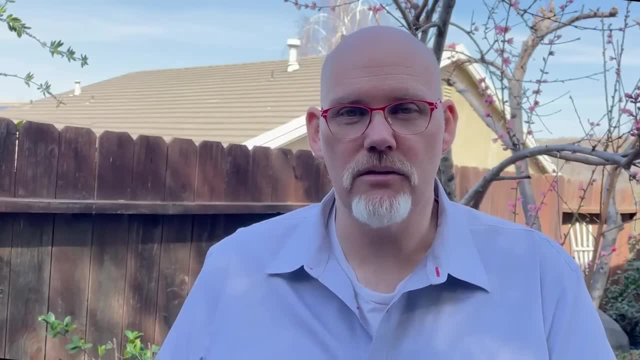 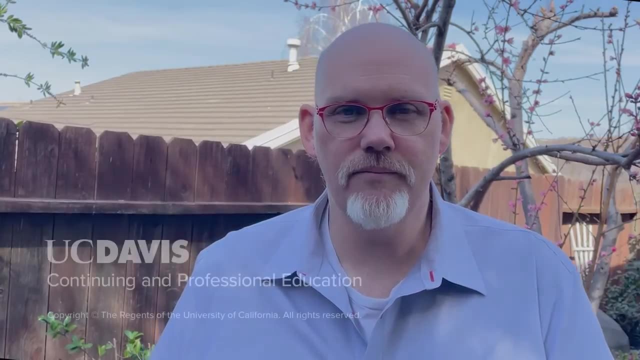 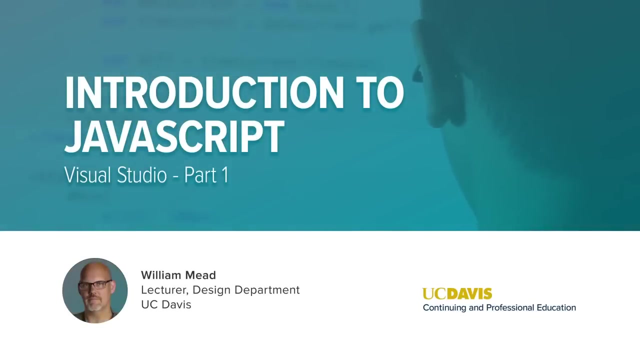 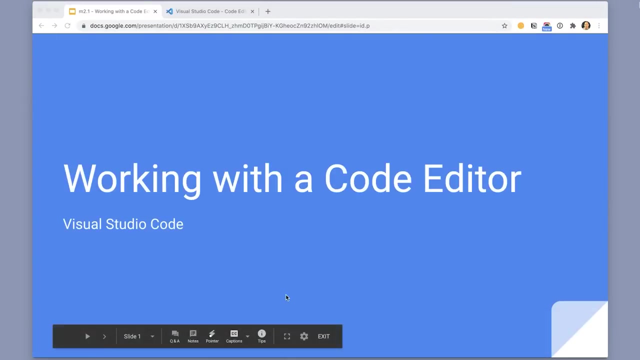 As much of that as you possibly can, because it will really help you learn JavaScript. So buckle up and let's go. This should be a really fun module for you to complete. In this lesson, we're going to be talking about working with a code editor, and I'm going to be specifically looking at Visual Studio Code, which I have a picture of here on this slide. 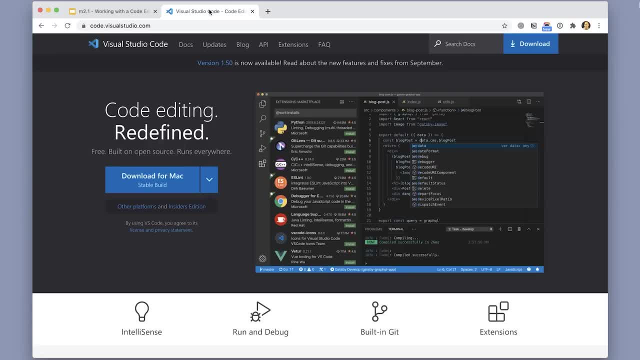 But I also have it open over here in this tab and you can go download Visual Studio Code for Mac or Windows for free and it's a great code editor. If you prefer to use a different code editor, such as Atom or Sublime Text or something else, that's fine too. 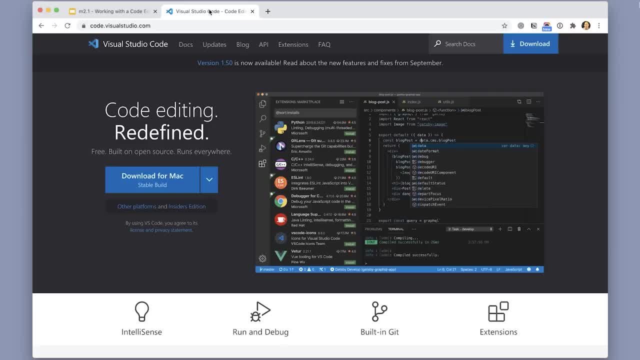 As long as it's got great features for editing code and it's not a word processor like Microsoft Word or something like that, then you'll be fine either way. But I'll be using Visual Studio Code throughout this course, So if you're interested you can go ahead and check it out. 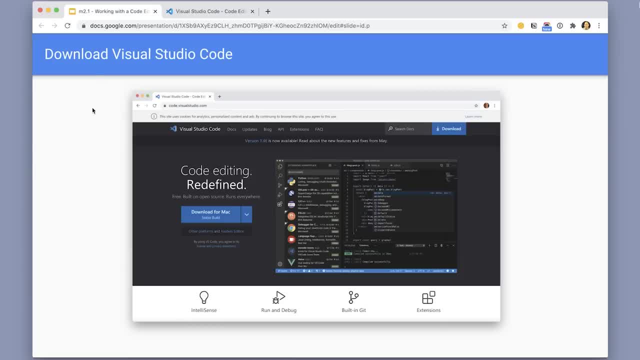 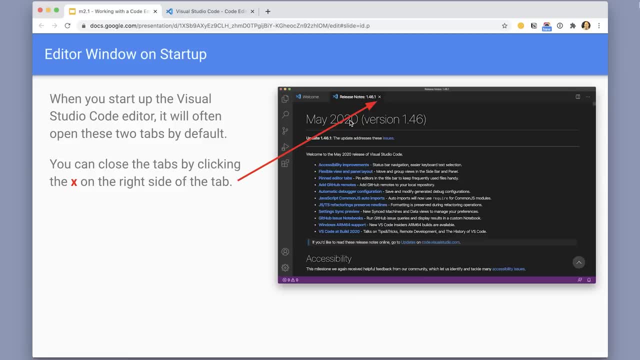 So if you're interested, you can go ahead and check it out. So if you're interested, you can go ahead and check it out. It might be helpful for you to use that as well. Okay, great. So sometimes when you open Visual Studio Code, you'll get these tabs open with a welcome or new release notes if they've come out with a new version. 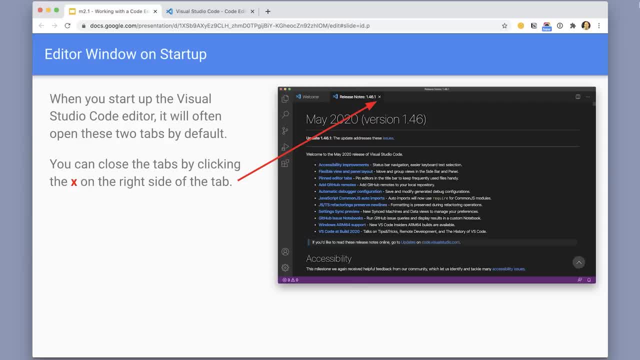 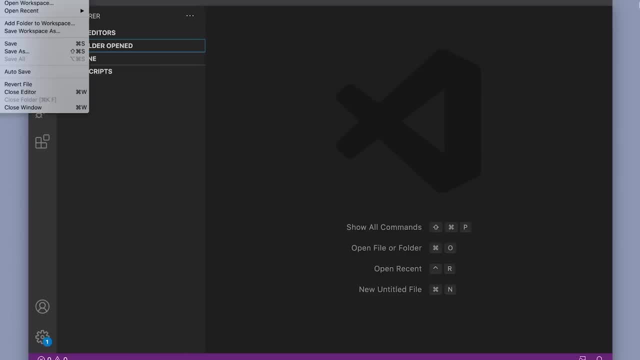 And you can just close those tabs by clicking on the X. You'll notice I have Visual Studio Code open and running here, but I don't have any of those editors open And I can make a new file by just going and choosing New File and that creates a new file on there. 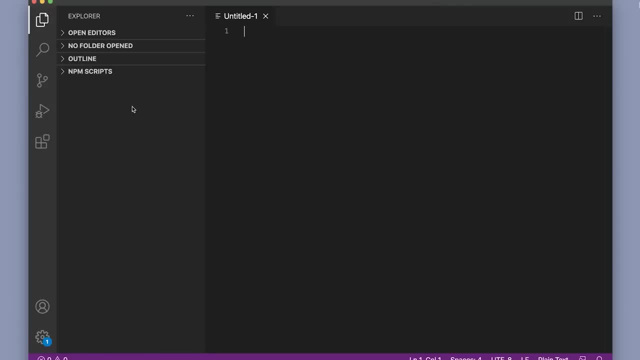 Now it's important with Visual Studio. It's important with Visual Studio Code that before you do anything else, you save your file. That way it knows what type of file you're working with. So I'm going to choose File Save As and I'm going to just save this as myfilehtml. 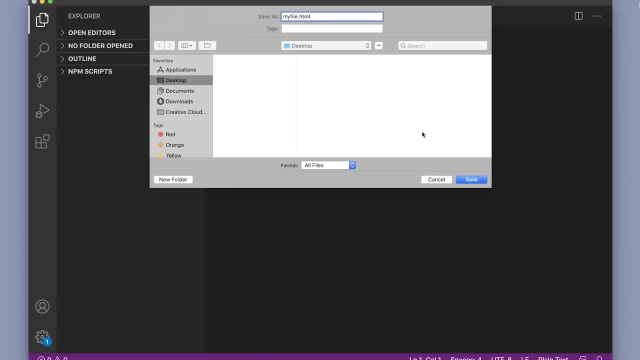 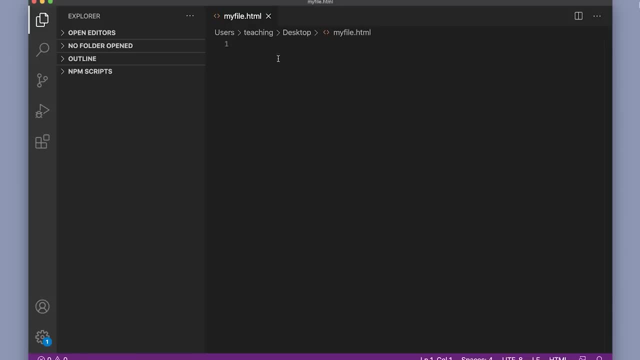 So I'm going to save an HTML file to begin with on my desktop. Once I have an HTML file, then I can easily get the basic HTML structure by holding down Shift, Pressing an exclamation point and then pressing Tab, and that will give me the basic structure for my page. 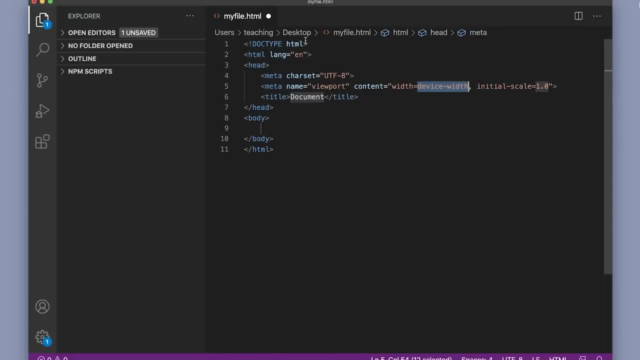 If you take an HTML class, you'll learn to type the doctype and to type all these tags, but we can use this shortcut. And again what you do to get it: just delete this exclamation point and then press Tab and then you can come in here and give your document a name: myfile. 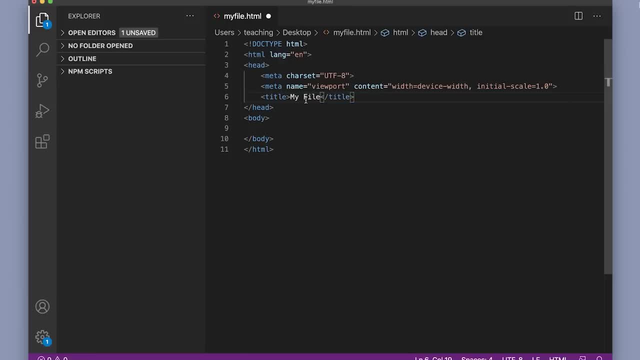 The title shows up in the tab. Okay, So that's kind of important. Great, So I can save that. Now one thing to notice really quickly while we're here: see this dot up here. That means this file has changed and it has not yet been saved. 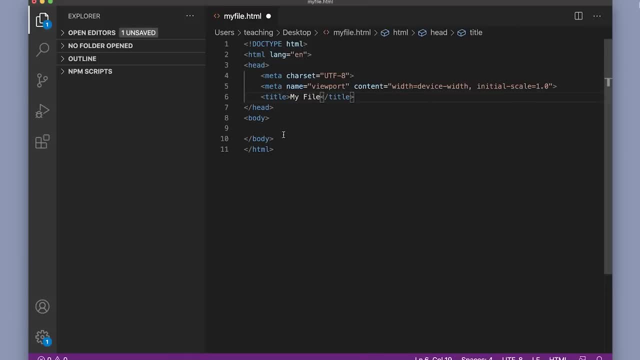 One of the frequent mistakes I see at the beginning with users getting started with working with HTML and CSS and JavaScript is they'll add things to the file and then they'll forget to save them. And then they go to run the file and they realize there are changes in the file. 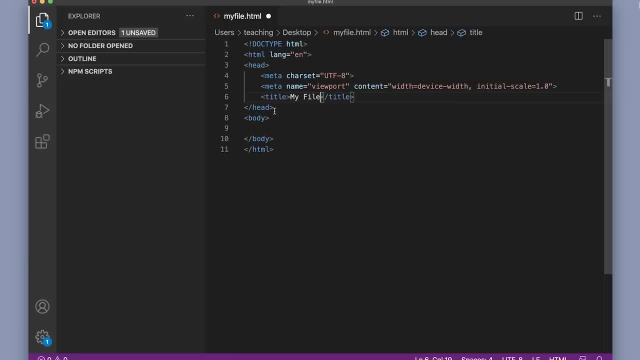 The changes aren't showing up. So watch out for that little dot. You can get that to go away by doing File Save over here or Command-S Control-S on Windows, and then it'll go back to just the X which you used to close that tab and close that window out. 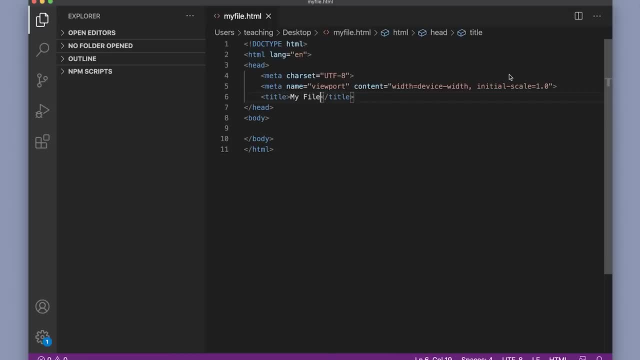 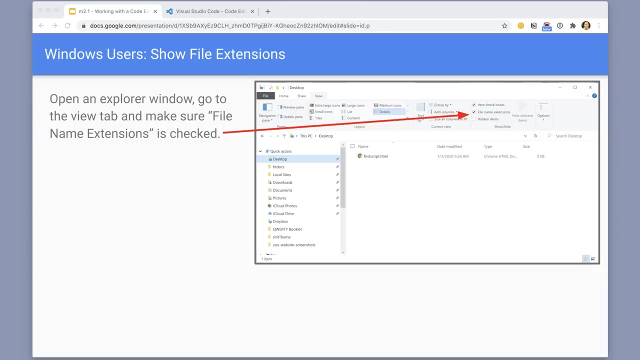 And then I can open this back up again by dropping it here and that will open that file back up again. So that gets me some basics of getting files open and working here In Visual Studio Code. A really important note if you're on Windows is open up just any Explorer window and click on the View tab and then go over and check the box that says File Name Extensions. 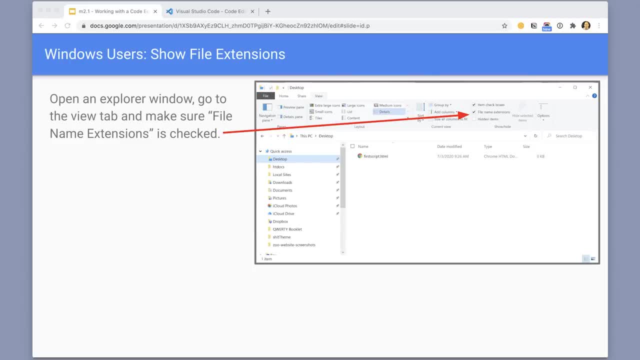 That way, when you save your files, you'll see the dot HTML file extension, And that's really important. Too many times I have students Making files that say myfilehtmlhtml And that's largely because Windows hides those file extensions by default. 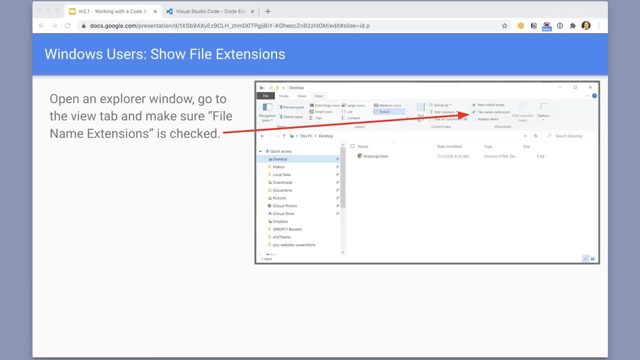 But we really want to be able to see them. It's really important to be able to see them And I show you this on my Windows laptop. but my Windows laptop has a terrible sound card and recording It just doesn't work out very well. 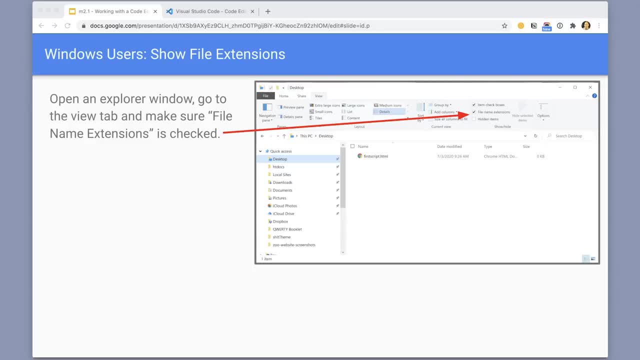 But here I have a screenshot of it. So please make sure you do that. Also, make sure that when you save files, make sure that the file name is always lowercase and never has a space in it. So I have myfile all as one word here. 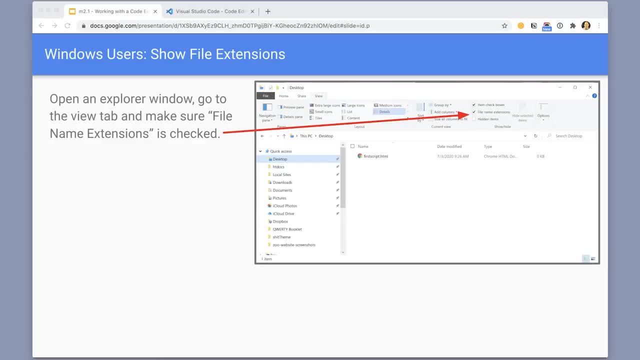 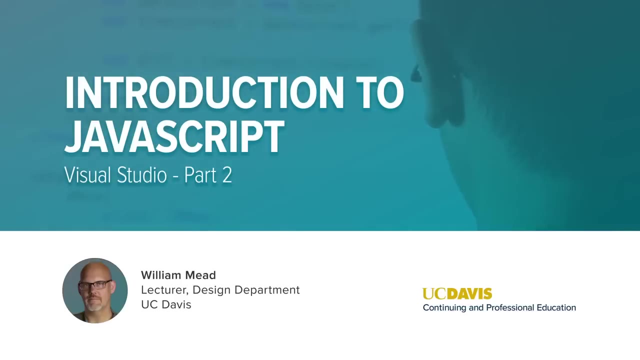 Do not put spaces in file names. I cannot be more explicit about that. Please do not put spaces in file names. It'll really cause problems for you. I'm back in my code editor And now I'm ready to add a script. 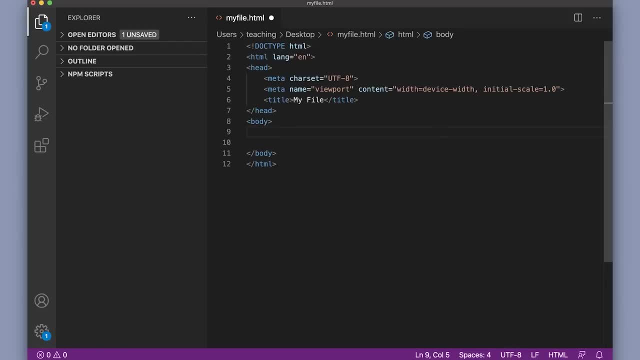 So let's add a script to this file And we can see some JavaScript actually happening here. First I'm going to put some HTML on the page, My first script- Nice, if I spell that right- And then you can actually put scripts really anywhere inside this file. 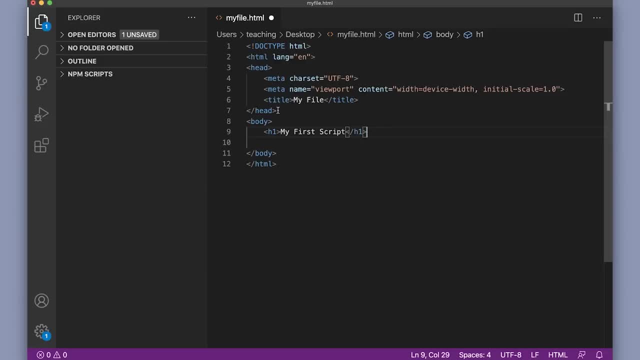 Sometimes they go in the head of the page here inside the head tag. Frequently you'll see them down here just before the closing body tag. So I'm going to make a script tag. Make sure you spell it right: Script. Look at that. What a mess. 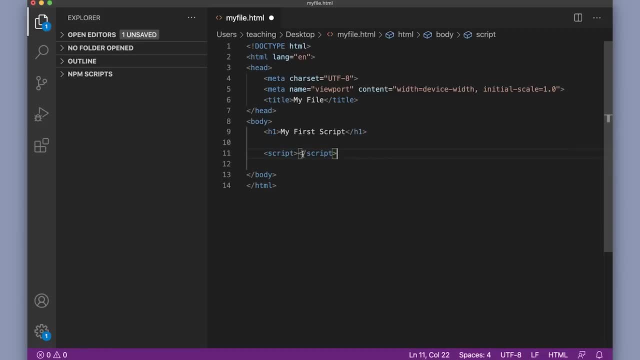 I'm going to make a script tag, So I have a script tag And I'm going to click between these two angle brackets here and move that down. Maybe I should do that again, Just to make sure I get it right here, If that's confusing. 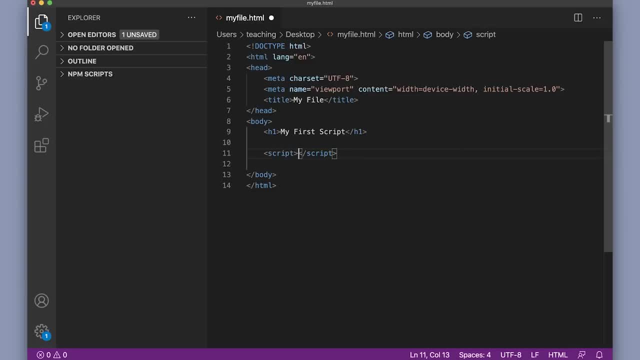 Script Like: so There we go, And then it puts the cursor between the two and I can move that down, And here I can make a variable var. hello equals good morning Bill. And then, in order to get it to do something, currently what we have to work with is the console. 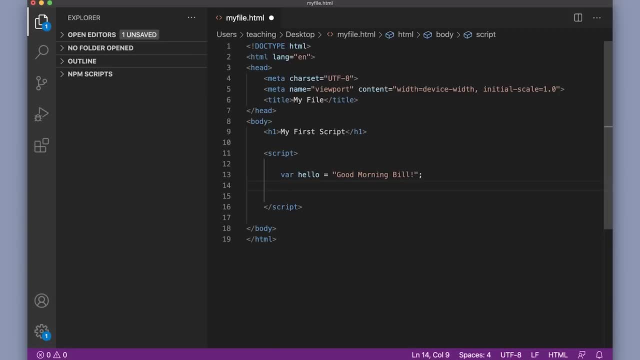 Because that's what I've shown you so far in the other videos. We'll get to other things later And really pretty soon. But for right now we just have the console, So I can use console dot log. Remember we talked about this method before. 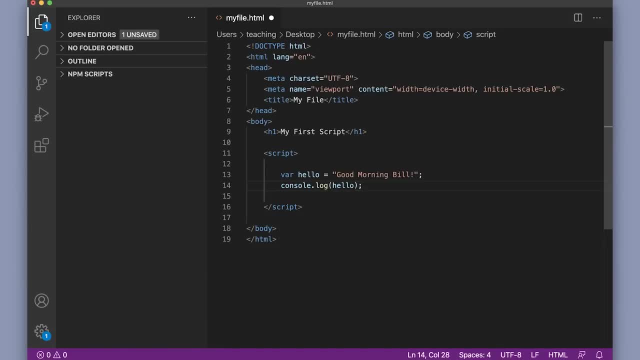 Hello, To put that variable, Or really the string associated with that variable, into the console. So I can save this file. Notice the dot up here. I have to save it. I can save the file And then I can go over to Chrome over here. 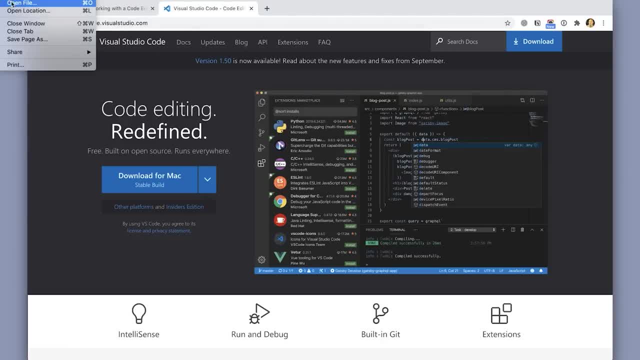 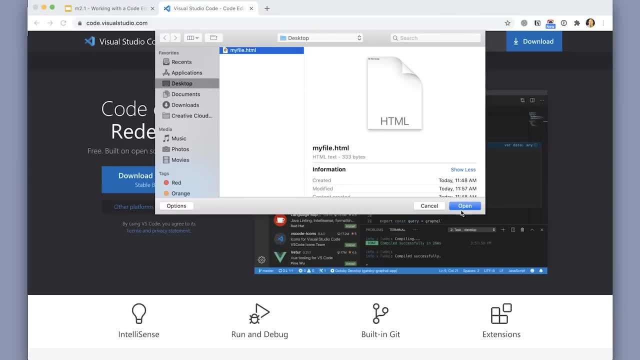 And I can go to file and open Where on Windows you can do command O. And then here I am on my desktop And I can open this file And it comes up And it doesn't really look like much, It's just a web page. 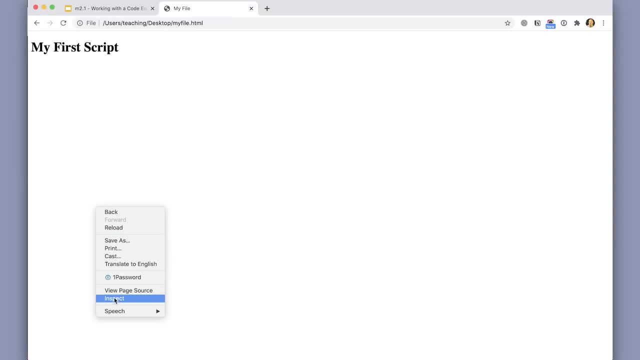 And we're not even seeing the script run. But if we go and choose inspect And then click on the console, You'll see that it comes up here And my JavaScript is actually running And it's doing this. So that's actually working great. 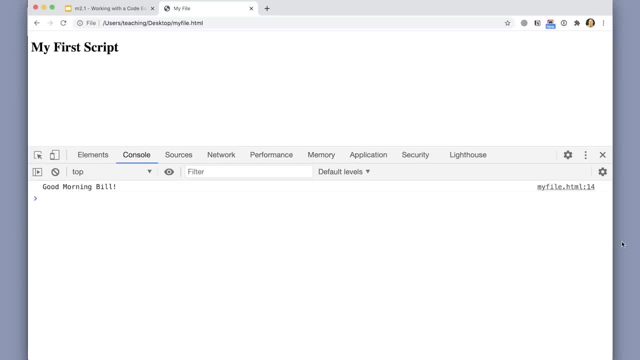 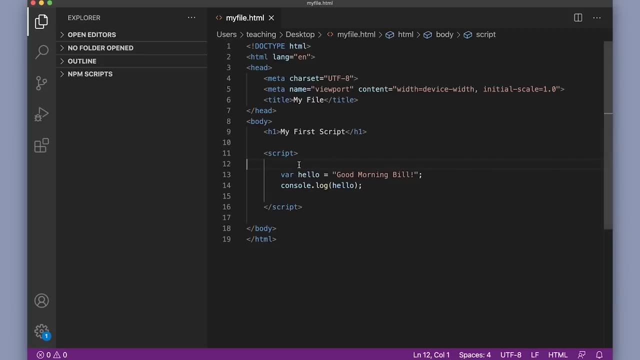 And really cool, We've gotten our first script to run. The next thing to talk about is how we can make some comments in JavaScript, And I want to remind ourselves exactly what we're doing. It's always a good practice to add comments to your scripts. 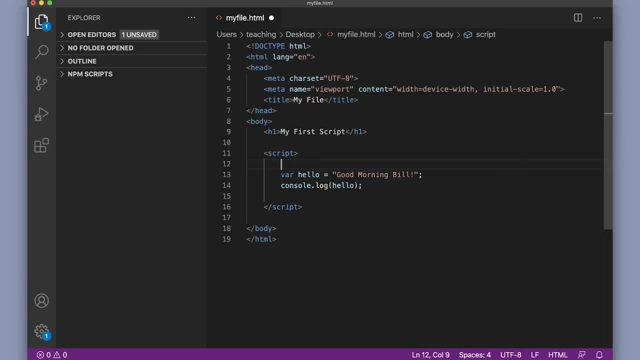 So that when you come back to them later you know what's going on. And there are two ways of making comments in JavaScript. I can use the slash twice, Two slashes, And I can type: the variable is below, Or something like that. 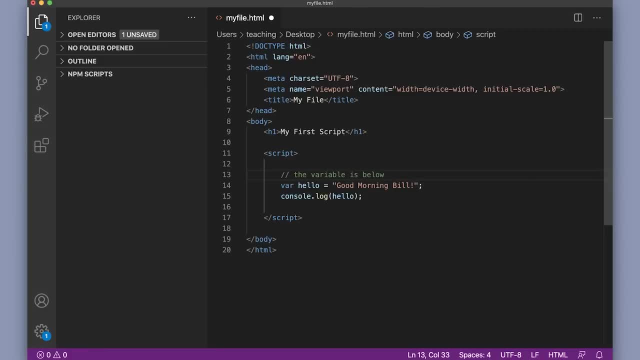 Or the variable below. We can say something else about it, But putting two forward slashes here will keep JavaScript from trying to do anything with this line here. If you want to have a longer comment, you can use the slash and a star And then end the comment with a star and a slash. 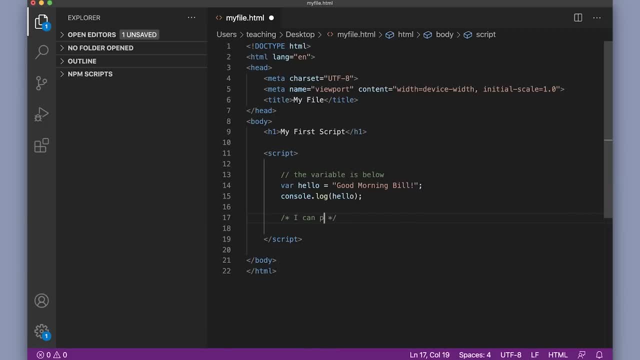 And then in here I can put a longer comment About anything So that I want, And it can go multiple lines, Like so, So I can have that start with a slash star and end with a star slash, And that will help me make comments in my code. 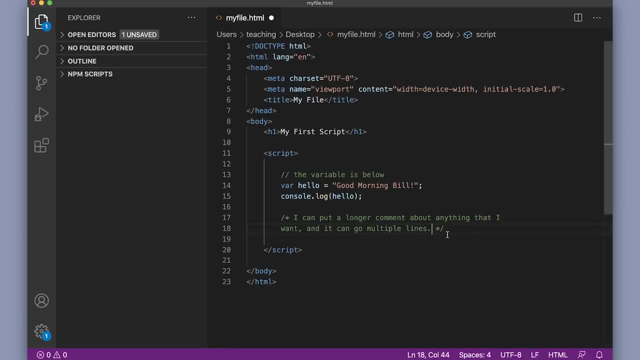 So that later, when I come back to try to find out what I was doing, I can leave notes for my future self, Which is super helpful. While we're here, another thing that's important is I can actually make the code in the browser larger or smaller by pressing the command plus or control plus on Windows on my keyboard here. 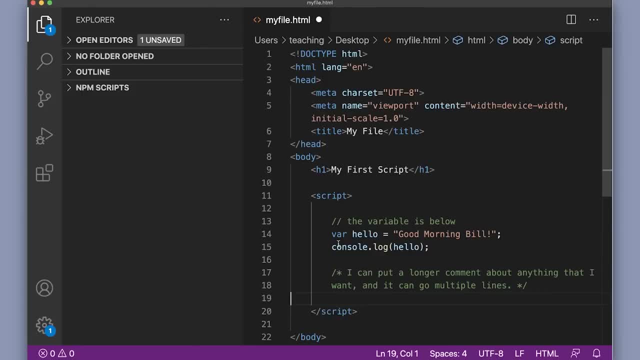 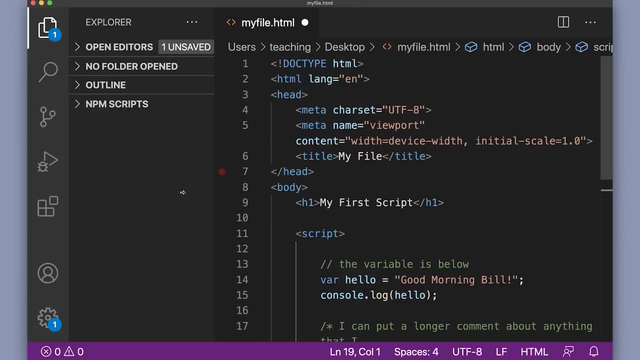 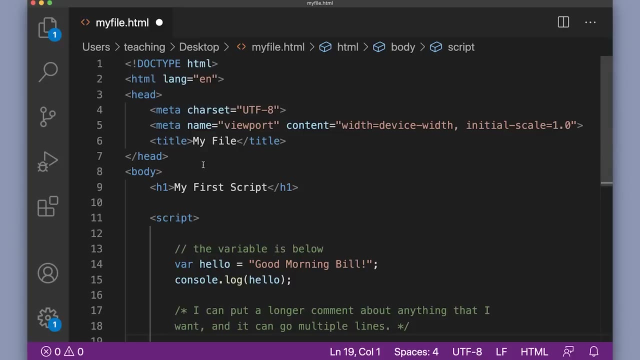 And that will make the code larger or smaller. And I can make this window over here smaller too. The code is getting squished in there. You can close it all together. This thing opens and closes that explorer, But I can make the code larger or smaller. 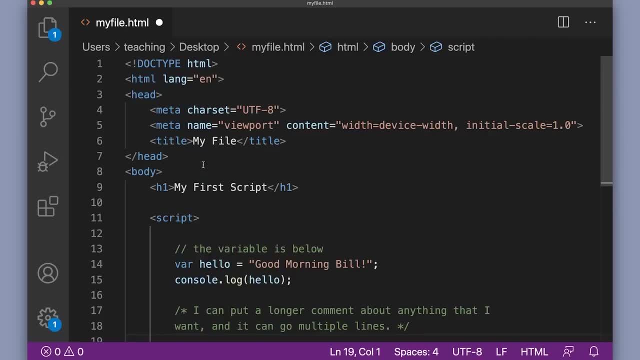 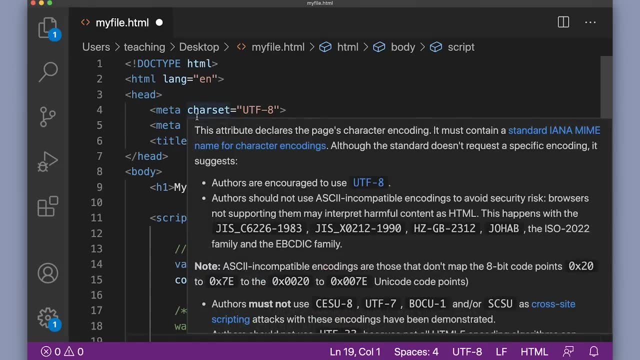 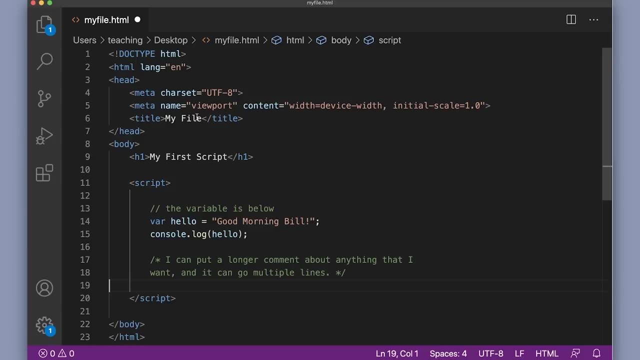 And depending on how good your eyes are, you might want the code to be larger or smaller. Command zero will put it at its default size, But command minus will make it smaller. So make sure you're setting your code to a size that's comfortable for you to read. 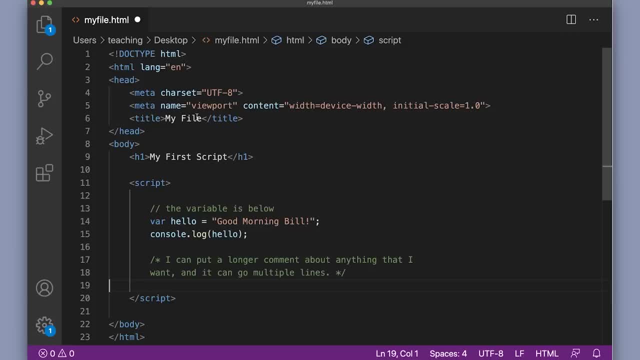 Because a lot of times when you're writing code, you're going to want to make it smaller. A lot of times when I'm working with students, I notice that they're having a hard time seeing the difference between semicolon and a colon. 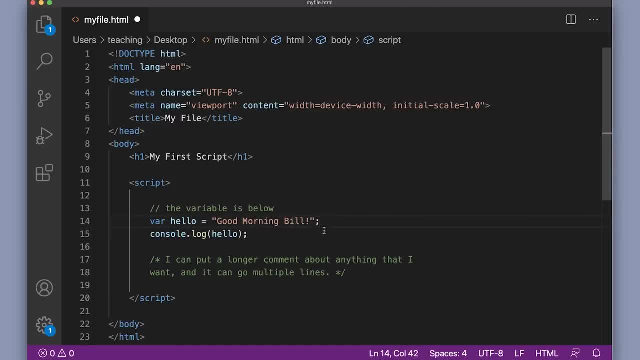 You know those are two different characters And if you're having a hard time seeing the difference between the characters, then the code is probably too small for you, So make sure you set it at a comfortable size. Thank you, Thank you. 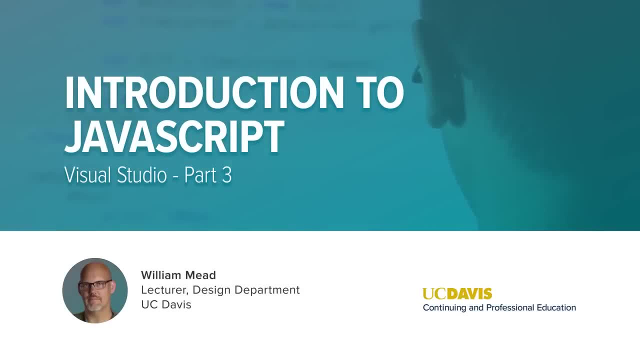 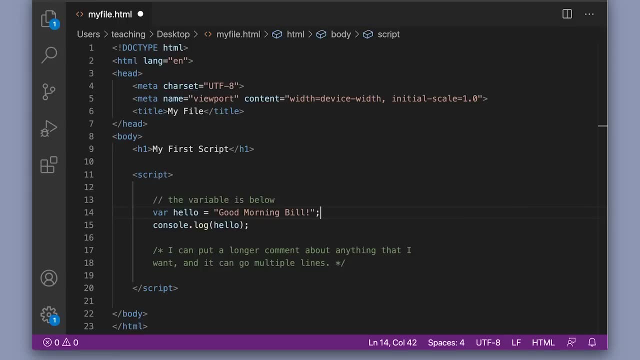 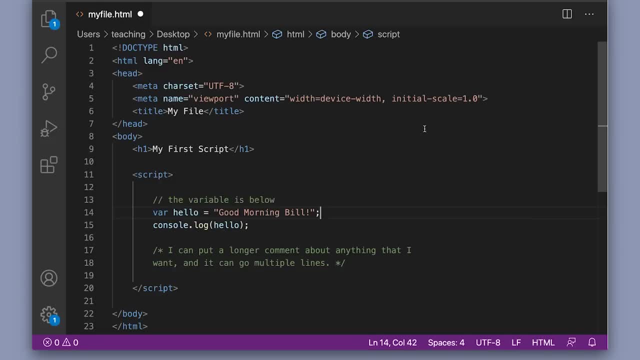 But usually if I'm working on a project, I'm going to have a folder with a bunch of related files. I might have an HTML file, I might have a CSS file, I might have multiple JavaScript files as we get going here, But for right now this is just a single file. 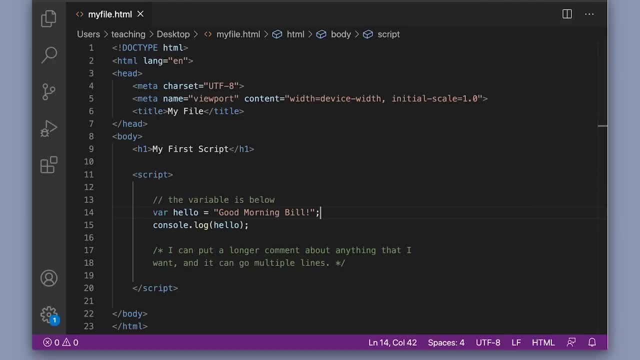 So that's not really very useful by itself. So over here I'm going to make a folder And I'm going to give the folder a name: myproject Notice. there are no spaces in that folder name. Never put a space. 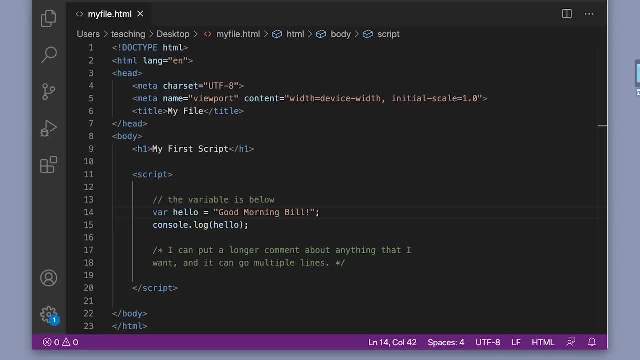 Also, all the letters are lowercase. It will just make your life so much easier if you keep everything lowercase. It doesn't have to be, But you have to not have spaces. So myproject, And then over here I could open up this sidebar. 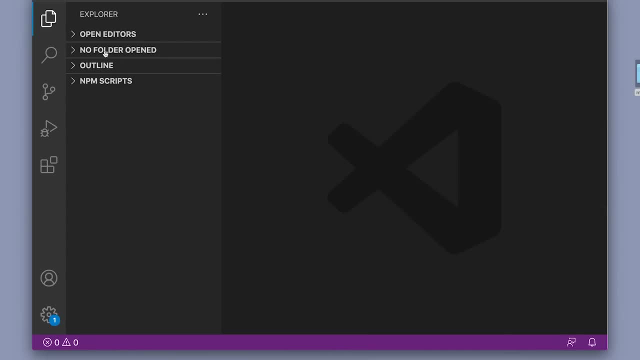 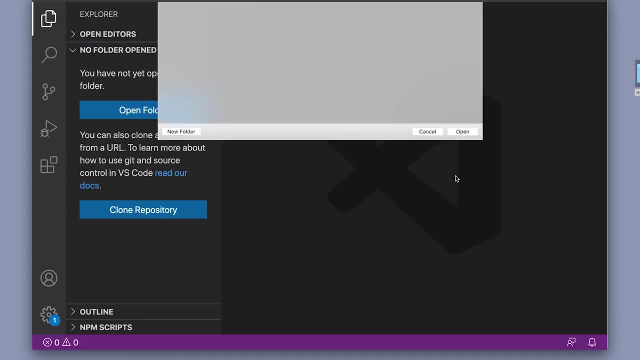 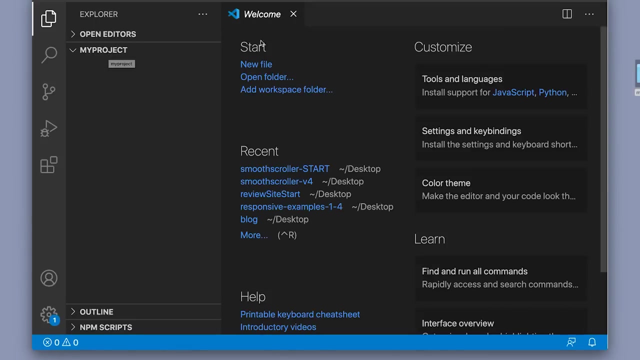 I'm going to close this file and open up this sidebar here And no folder opened. I can actually open that folder, myproject, And now you can see I've got my welcome screen again And I've got myproject here, And there's no files in this folder currently. 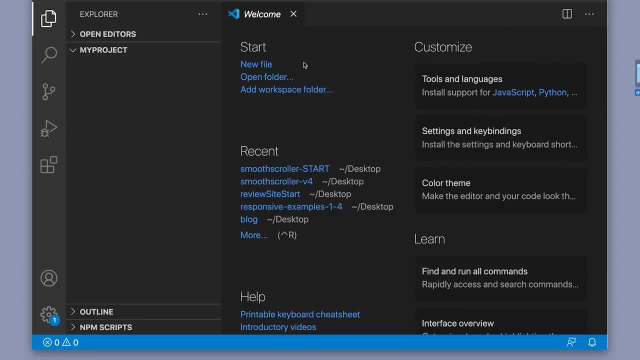 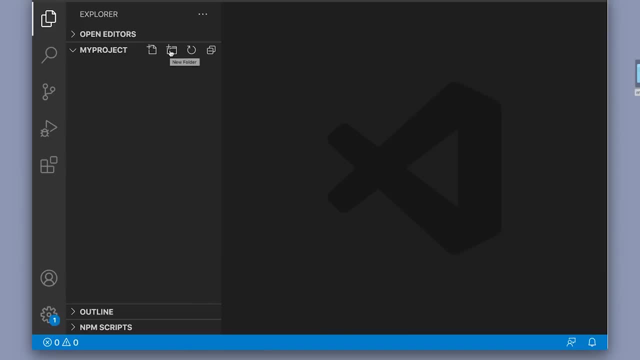 I just made a folder and it's empty. But I can put a file in that folder. I'm going to close that welcome screen Over here. this button will create a file. This button will create a folder. Be sure you're not confused between the two. 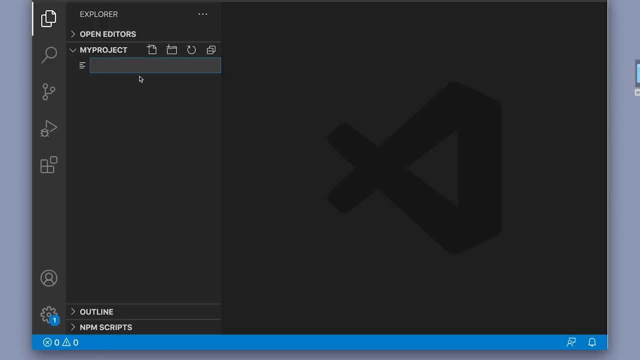 So if I make a new file, suppose I make a file and call it indexhtml. That's going to be an HTML file And I can put that in my folder. And now you'll notice it's created the index file. And not only that, but if I look in my project folder over here, 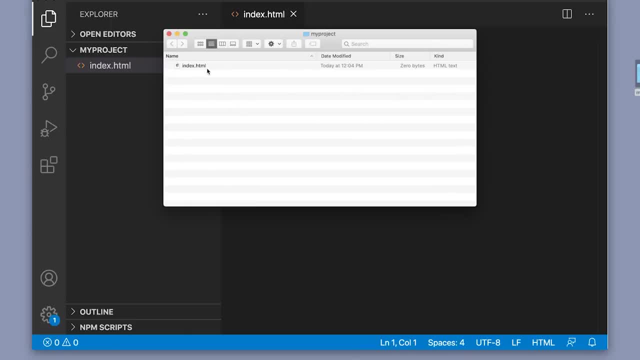 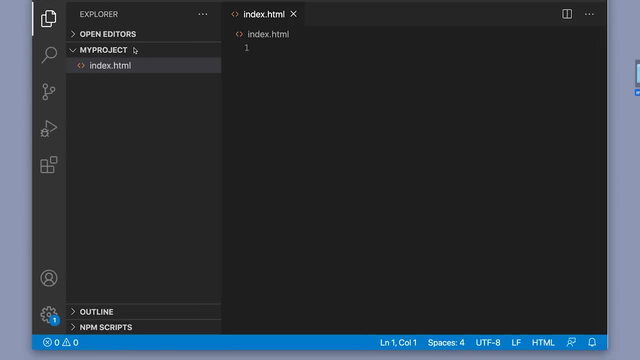 you can see that indexhtml has been created in that folder, And so I can manage my whole project from here. Perhaps I have another file in here. I'm going to have stylescss, So maybe that's going to have some styles for my web page. 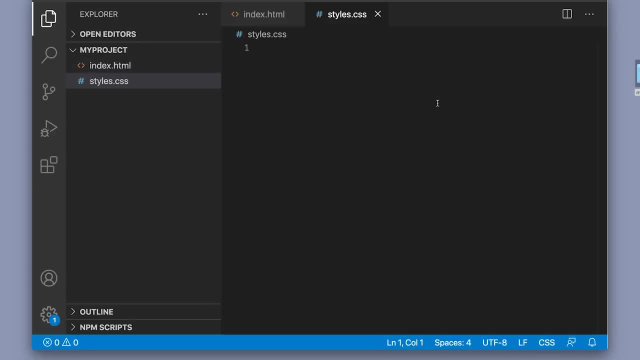 And it's going to go into that file. So now that file is now in the folder over here And in this way I can control and keep track of all the files for my project, and they're all in one place. Remember I said earlier: 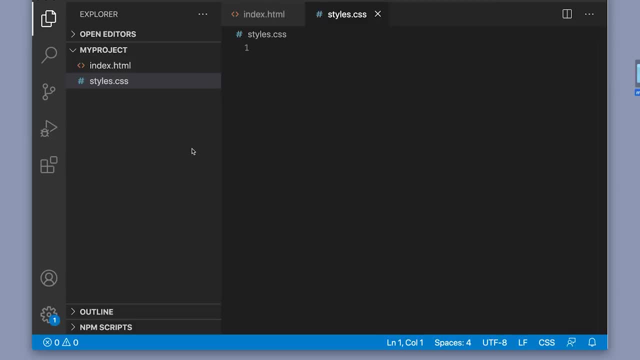 you have to get really good at file management and you have to make sure that all the files for a project stay in the folder And you might have other folders in the folder. So if I come back here I might make a folder for images. 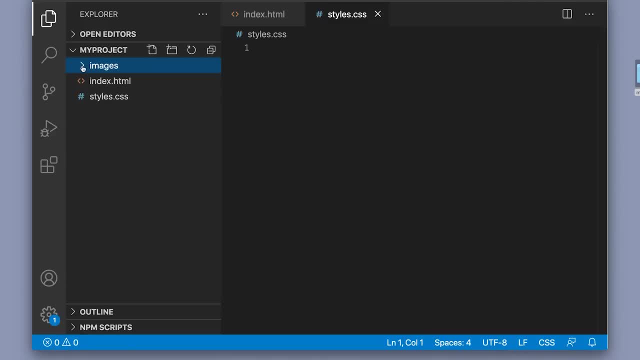 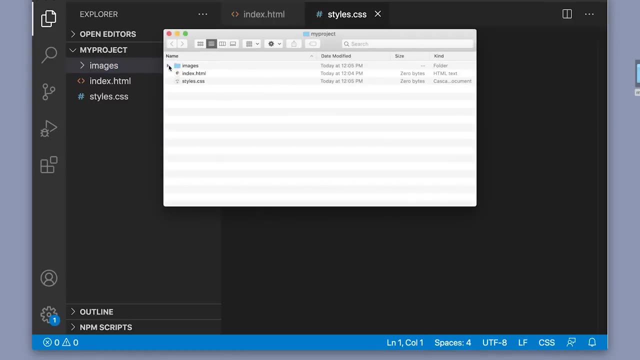 Now, this is a folder And currently there's nothing in the folder, But if I look in this folder over here, you can see that the folder images is here And I could put images in there. Be careful when you're creating files. 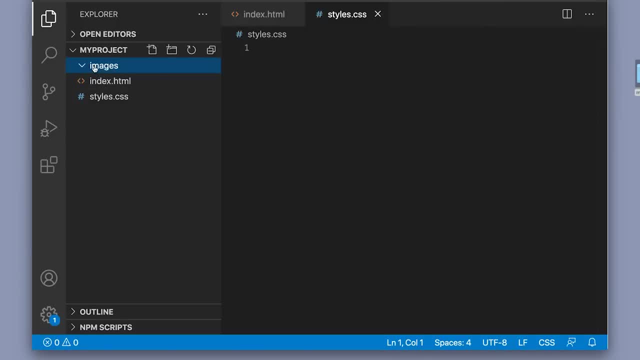 not to accidentally put the file inside the folder if you don't mean to. So if I click new file here, it's going to create this file inside of images Oopshtml. So this file is actually inside the images folder here And I can see it over here as well. 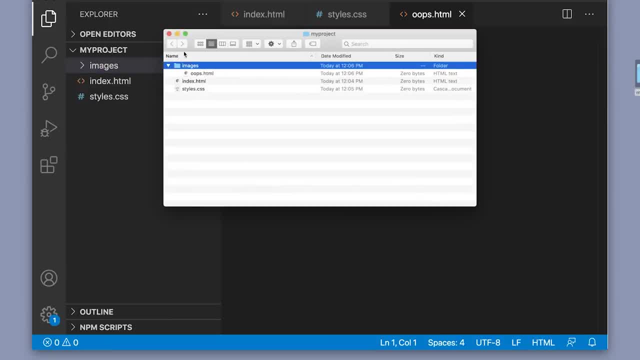 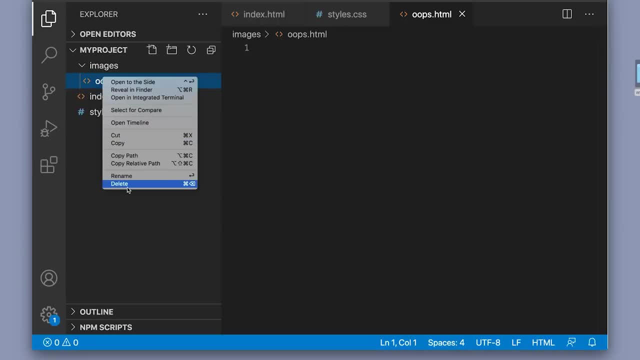 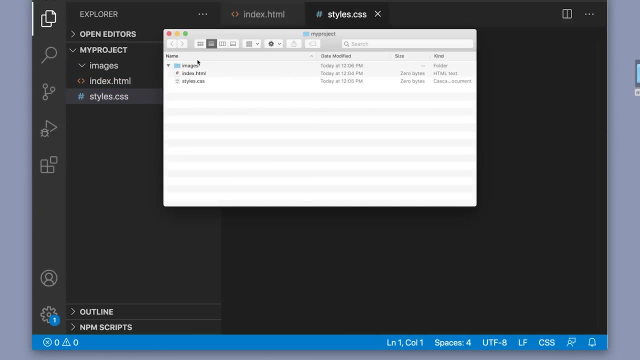 As being inside the images folder. If I decide I don't want that file, I can right click here and choose delete. It'll ask me: do I really want to move it to the trash? And sure enough, from over here, that file is now not inside that folder. 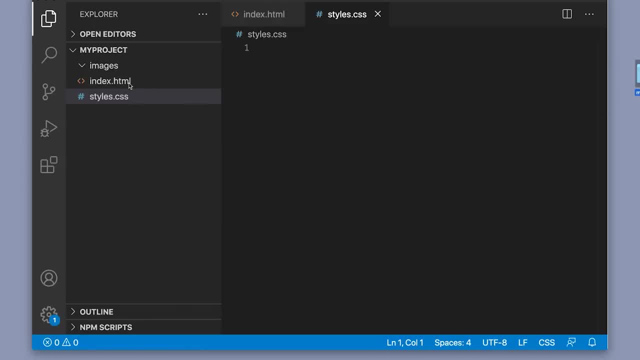 The folder is empty again. So by working with this explorer over here, we can create files and manage files for our projects and make sure that they're files are in the correct places at all times. The last new thing that I have for this lesson is: 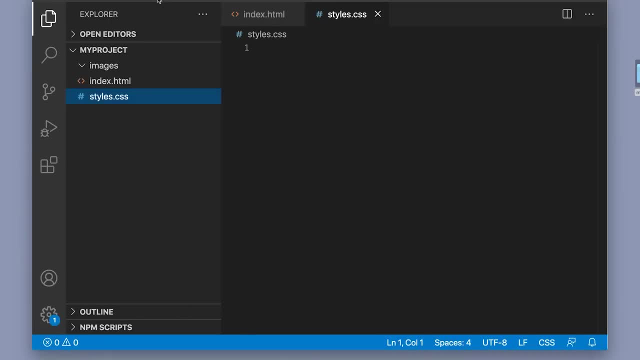 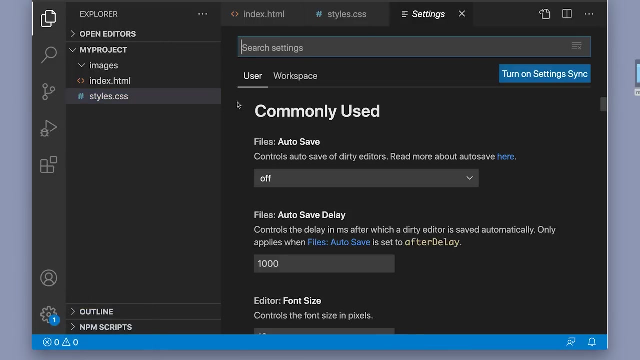 I just want to show you that Visual Studio Code is very customizable. You can add all kinds of extensions to it, And if I click on this gear icon down here I can get into the settings And I can do all kinds of things. 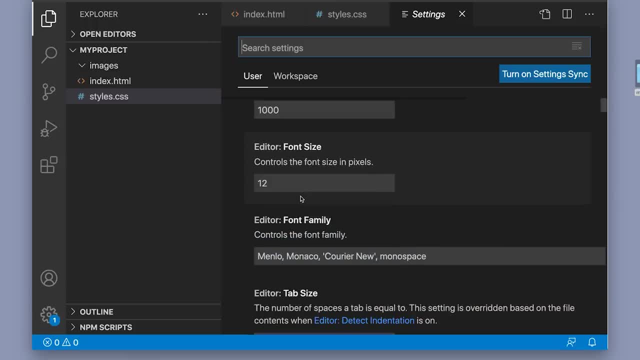 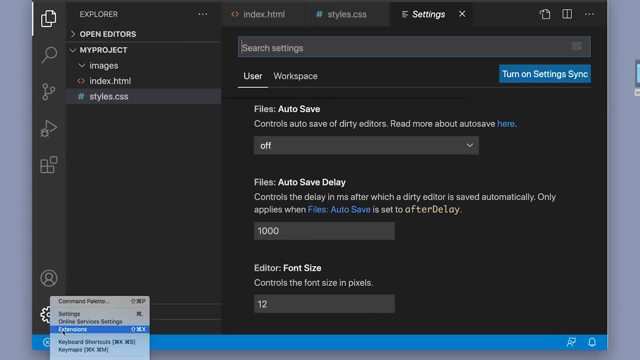 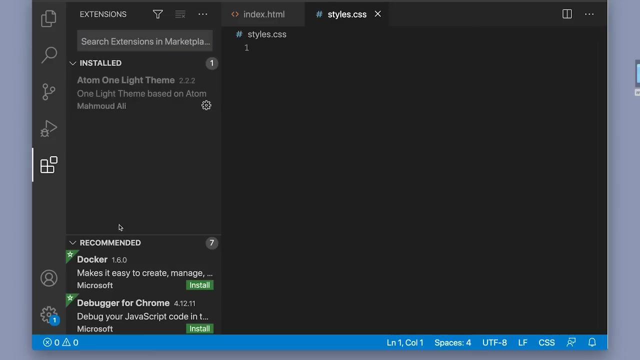 I can add all kinds of things in here With extensions and other kinds of things. So, for example, you can search for settings or extensions. Here are extensions here. Not sure about the settings, But you can do all kinds of fun things to make. 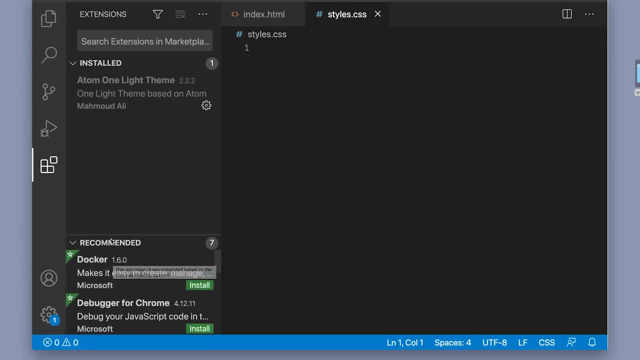 to make Visual Studio Code more, more personalized. Maybe you like this black look for your code editor, Or perhaps you prefer a lighter theme. I installed this extension here called Atom One Light Theme, And you can click on that, And currently it's disabled. 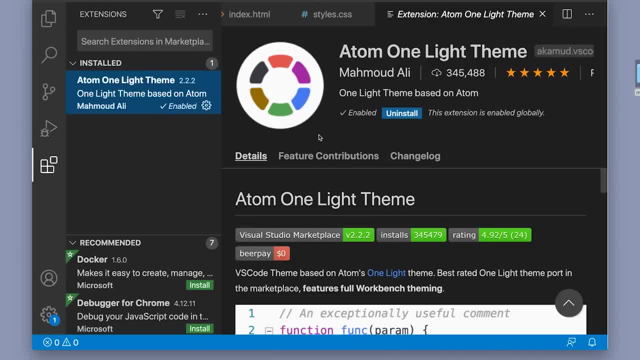 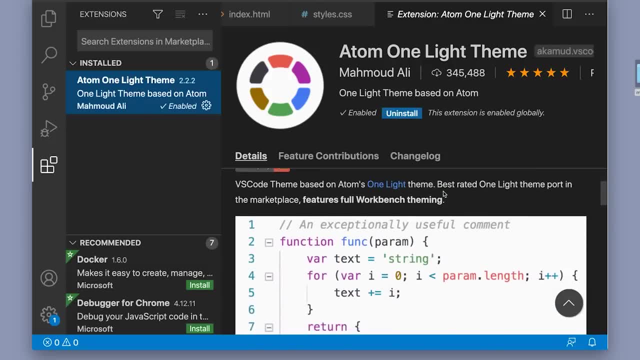 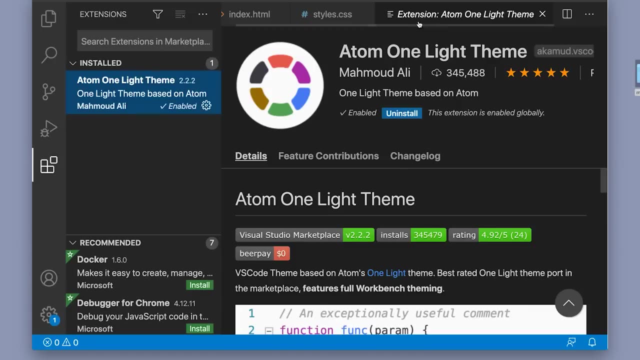 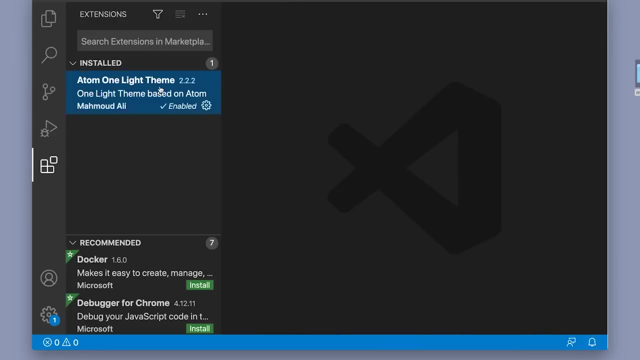 but I can enable this theme And I think down here should be able to choose feature contributions. It should be switching here. Not sure why that didn't switch. This happens sometimes. Oh, select color theme, There we go. So here I've got the color themes. 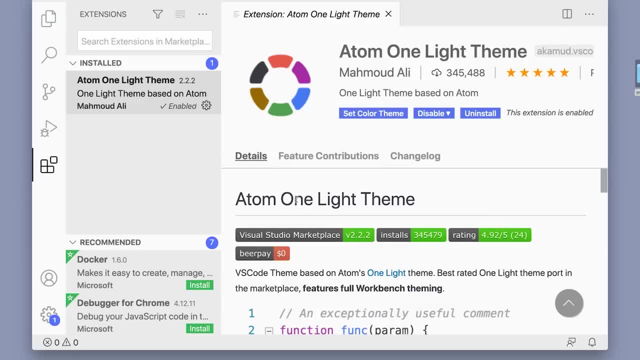 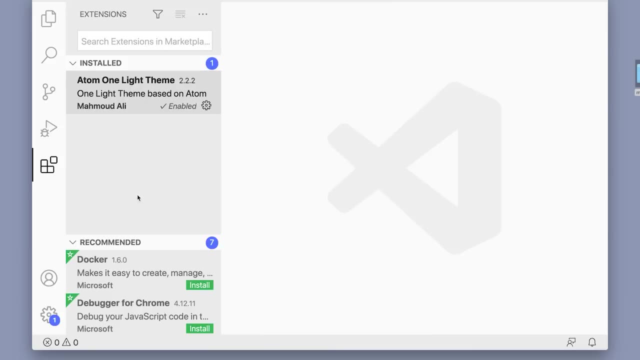 and I can select Atom One, Light. Sometimes you have to mess around with this, extensions and the theme editor and the settings to sort of really figure it out. But there's all kinds of themes that you can get for Visual Studio Code to customize it and make it look the way you want it to look. 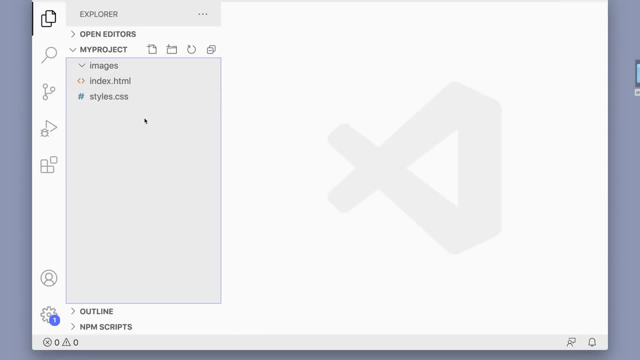 And I can go back to my files. And here I am, And so now you'll notice that my files will look a little bit different because I'm using the Atom One Light theme. So yeah, So just to just to remember here. 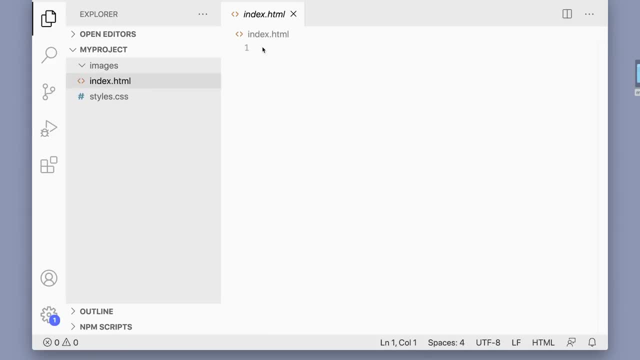 we've done quite a lot to to make this, make this page. Whoops, I don't know why it's not letting me edit my file To make this page different. here I'm going to redo that last part because I kind of messed that up a bit. 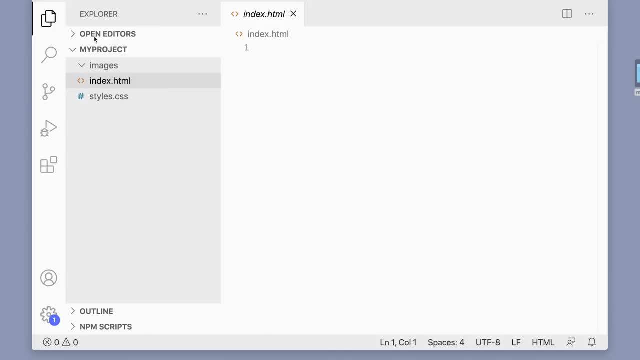 So you can see here I am in my project again for my index file And I can come over here and click And just to review what we did in this lesson I can type an exclamation point and press tab to get the basic structure of the page. 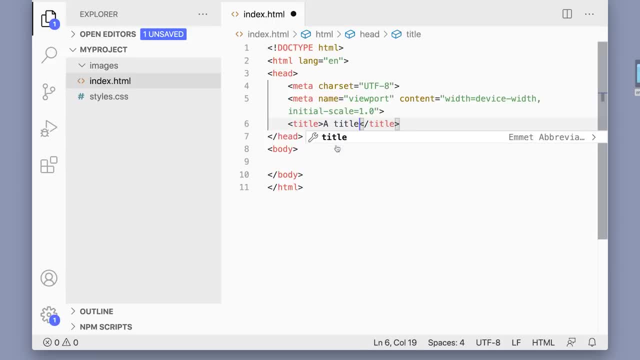 And I can add a title for my document here that will show up on my page. I can add some HTML. I'm just going to add an H1.. Here is a heading, And then I can add some scripts. I can add some script tags. 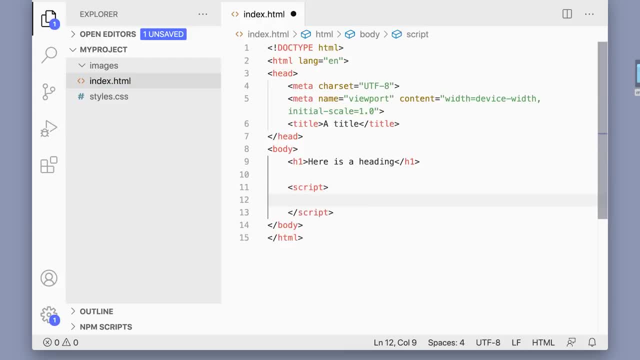 And I can add a script to my page. So I could do something like bar my variable And set it to hello, And then I could console log out. Console dot log my variable. Notice it pops up here. I can even just press. 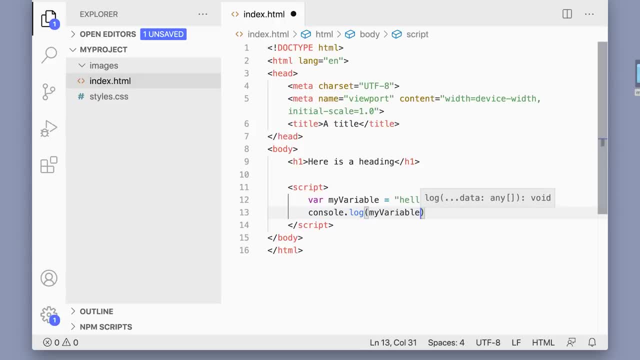 I don't even have to type the whole thing, I can just press return to get it to pop that in place. so I make sure I don't spell it wrong. And then a semicolon. Semicolons are used in JavaScript at the ends of statements. 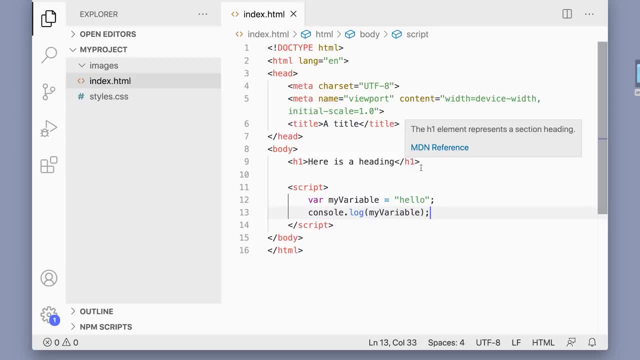 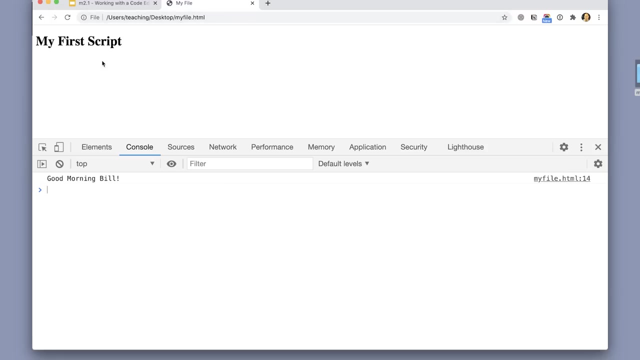 I can save that file And then I can come back to the browser and test it. Let's do that really quick. Come back here to Chrome. This is the other file. So I'm going to open this file. I can do command O. 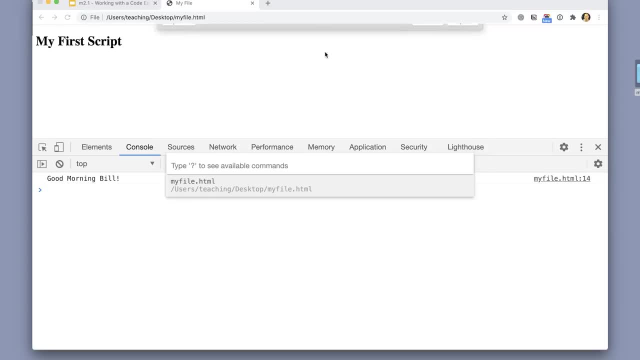 And there we go, My project index. And there it is, And it's doing hello there. So the hello came up in the console log there. So that's a review of everything we learned in this lesson. You're now able to work with files. 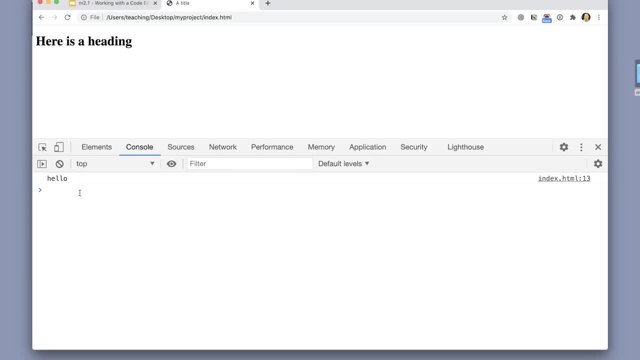 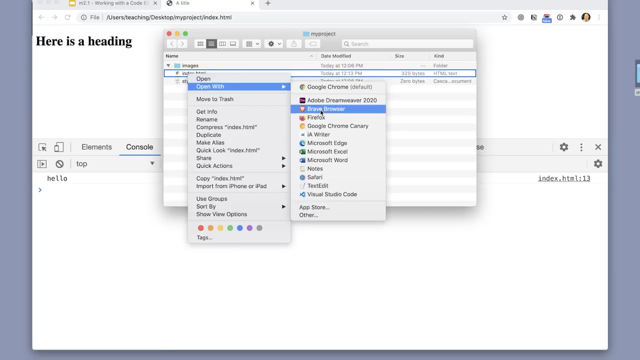 and get those files to output content into the console that you can then test in your browser, And that's a great way of working. Another way of opening your file is to right click on the file and choose open with and tell it to open with the browser. 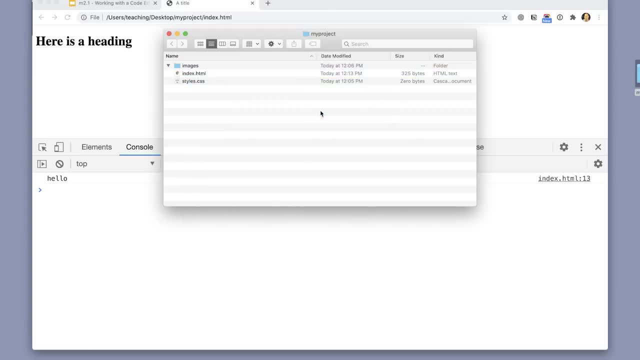 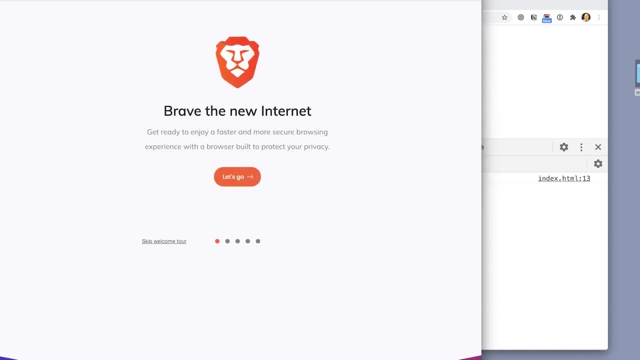 You could even try a different browser. Brave is a great browser to try. Brave is using the same rendering engine as Chrome, so it actually works the same way as Chrome generally. But what's interesting about Brave is that the CEO of Brave is actually that Brendan Eich guy. 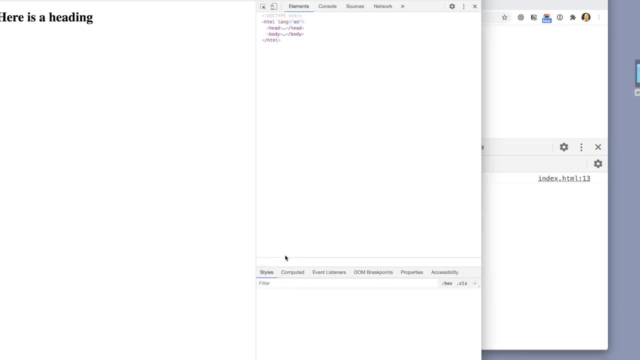 who invented JavaScript. So it's kind of interesting to note that the guy who invented JavaScript is now in the business of creating a browser. So that's kind of interesting. Okay, great, This will get you started And I look forward to seeing you in the next lesson. 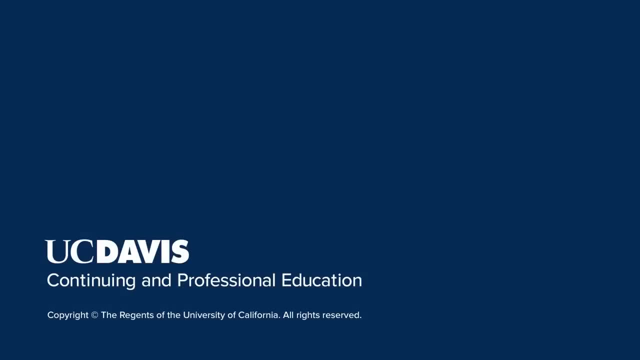 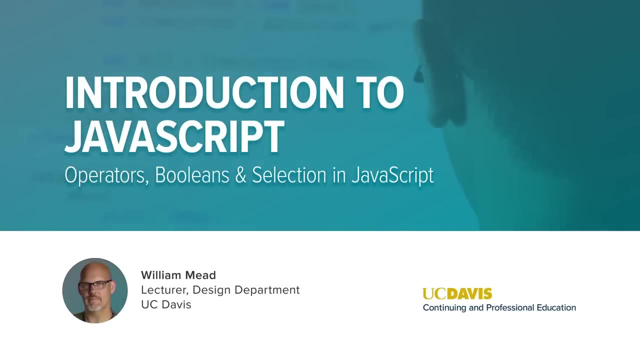 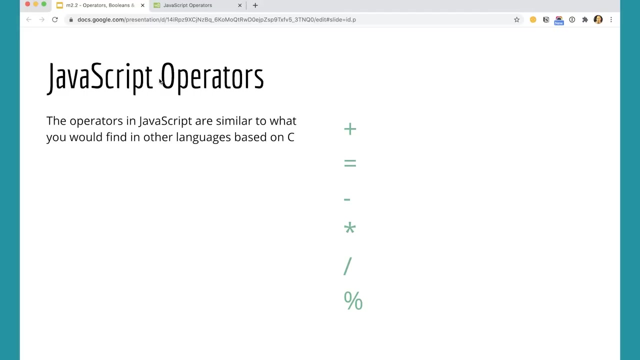 where we can start writing some interesting scripts: Operators, Booleans and Selection in JavaScript. Operators in JavaScript are the symbols that will allow us to create different expressions in JavaScript, And here are just a few of them. We've already seen the plus sign. 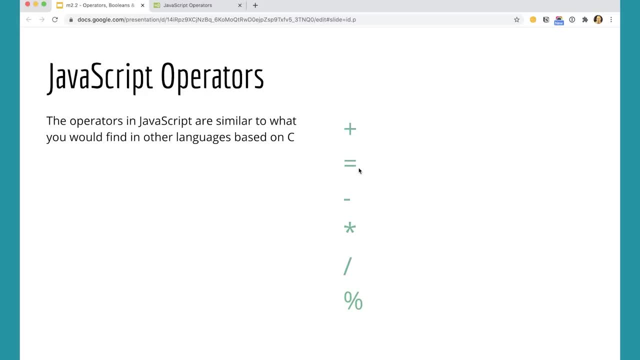 and the equal sign, which remember equals, is an assignment operator. There's also a minus, and the asterisk is used to multiply and the forward slash is used to divide And the percent is a modules operator. If you want to find out more about operators. 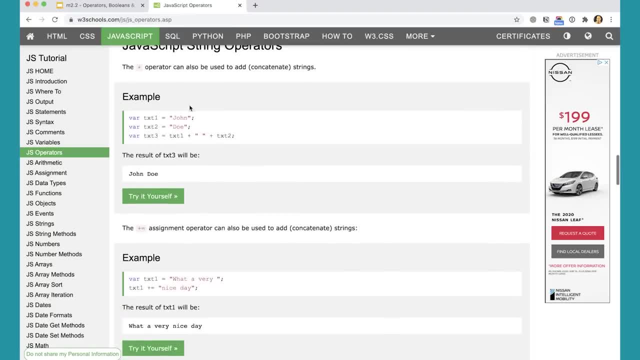 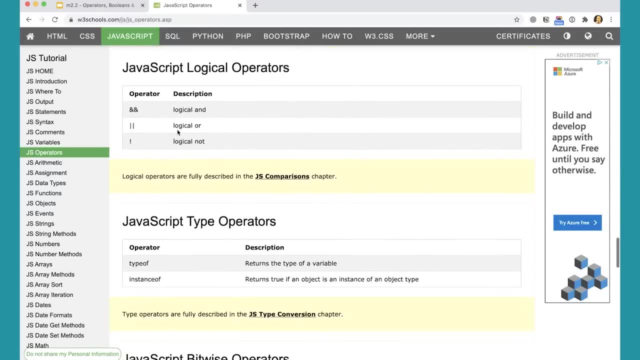 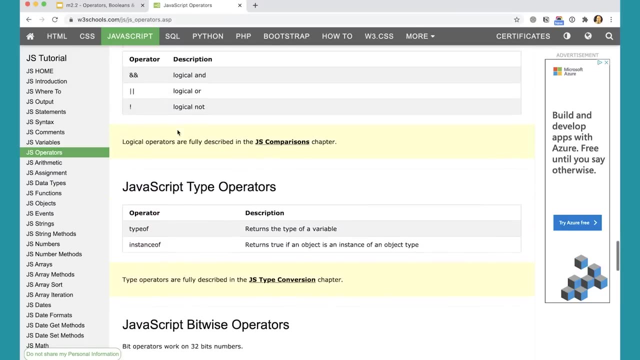 you can come over to the W3Schools website and look at the different operators. They'll get all listed here- Comparison operators and logical operators and all kinds of stuff here- So you can come through and find all the details about all of the different operators. 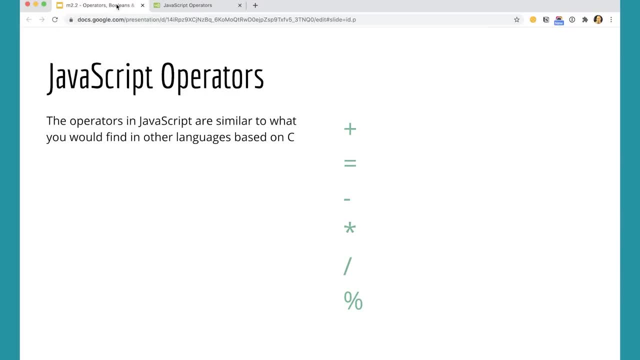 if you want to there. But we're just going to start with a few of them so that it's not too overwhelming, And most of the operators are very similar to what you would find in other C-based programming languages: C, C++, C, sharp Objective C, so on and so forth. 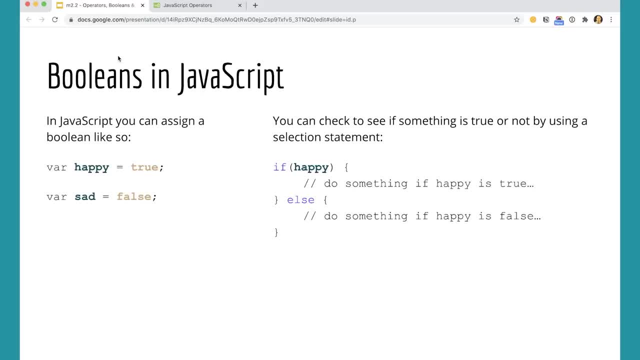 Okay, so there's also Booleans in JavaScript, And it's very nice to know that a Boolean can have two values: true or false, And that's it. So here I'm making a variable called happy And I've assigned it the value of true. 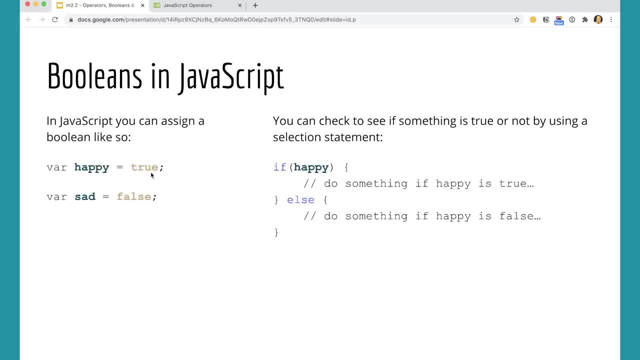 Notice that true is not inside quotes. JavaScript knows what true means. True is a keyword that means that something is true, And false is a keyword that means that something is false. So I have a variable here. sad It's false. I can use an if statement to check. 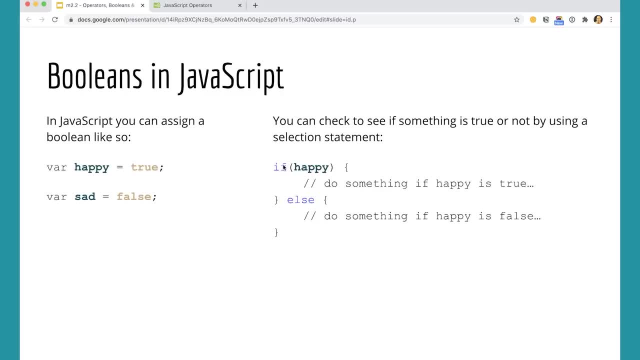 to see if something is true. So if happy. Now, happy has a sign in it And I've assigned true to it, So it's going to do something here. If I were to replace happy with sad, then the else would fire instead of the. if 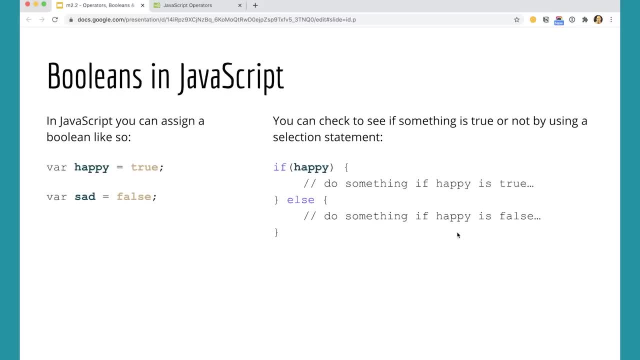 And we would do something down here if happy was false. Or if I change the value here from true to false, then happy would be false And it would do this down here. So that gets us started with a little bit of that. So next we're going to move to our code editor. 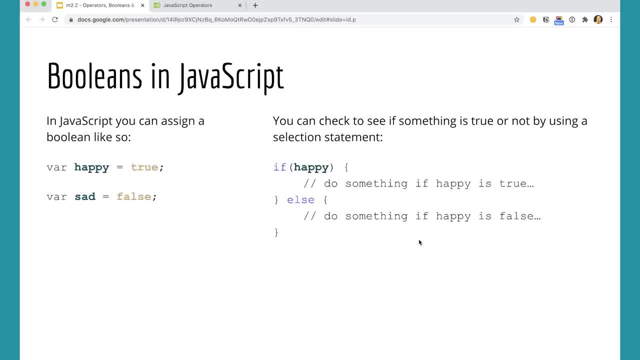 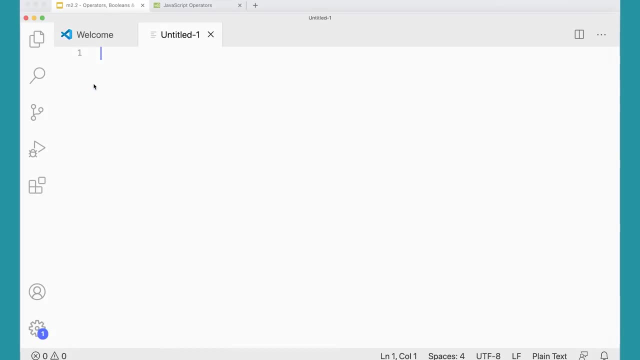 And make a file and try working with some selections and booleans and that kind of fun stuff. Here I am in my code editor And I'm going to make a new file. And I'm going to make a file. Before I do anything, I'm going to save the file. 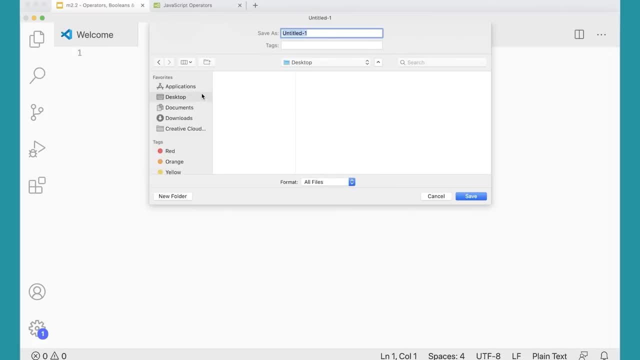 Save, And I'm going to just save it on the desktop And I'm going to call it: SelectionsHTML. Notice: all lowercase, no spaces in the HTML extension. I'm going to save that on the desktop And then again the exclamation point will allow me to press Tab. 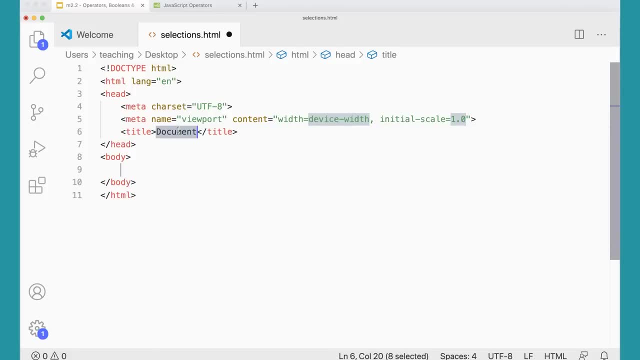 which gives me kind of my basic structure for my HTML page, And then I'm going to type in here testing selections And booleans. There we go, And then in here I'm just going to add an H1 testing selections. 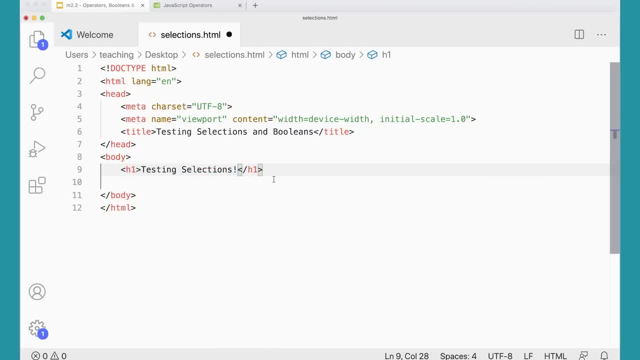 There we go, That's nice. And then I'm going to add a script tag, So we'll go ahead and add a script in here, And then what are we going to put in the script? Well, let's make some booleans. 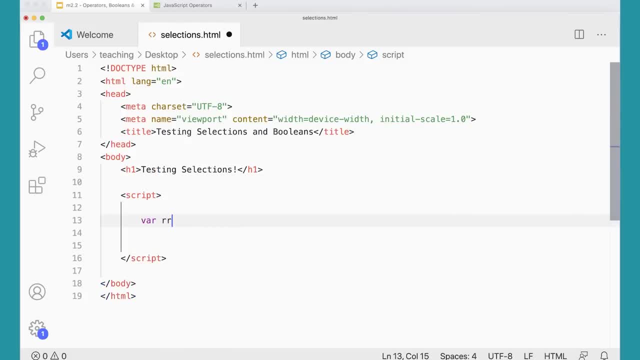 I'm going to have var red And I'm going to set that to a value of true. And then I'm going to have var blue And I'm going to set that to a value of false. There we go. So I've got two values here. 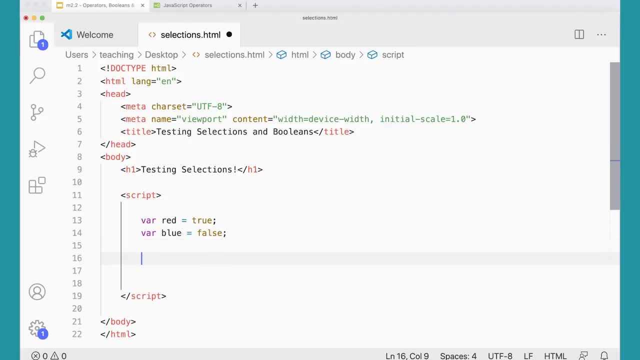 One is set to true and the other one is set to false. Now, if I were to make an if statement, if parentheses and I were to check the value of those red, I'm going to check the value of red. 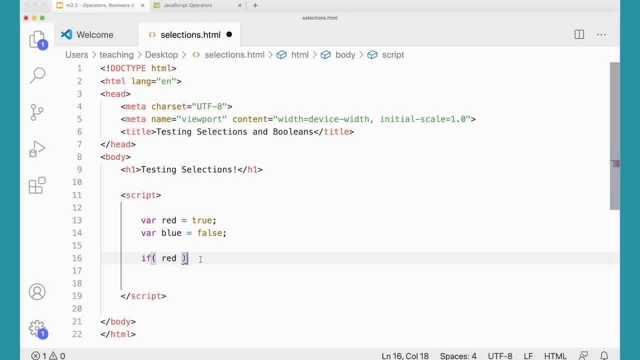 If red is true, which it is- then something's going to happen here. Something happens. Red is going to evaluate to true, because I have true assigned to the red variable here. If I were to put blue in here then this would not be true. 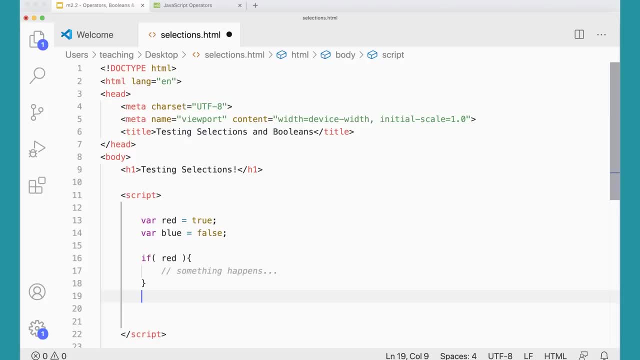 in which case something else would happen. So I'm going to come down here and add else. Now this else statement. sometimes you'll see it up on the same line, like this, And sometimes you'll see it on the next line, like that: 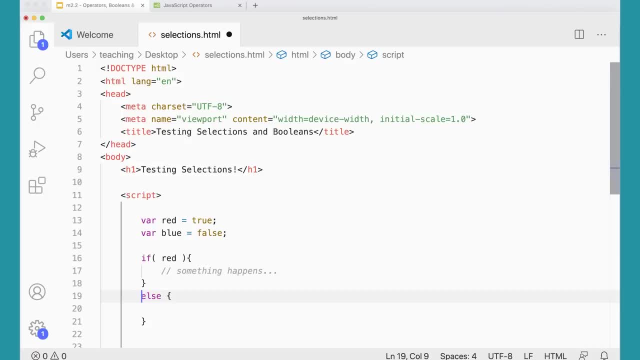 That doesn't really matter. That's a styling choice. Some people like to keep their code a little bit more compact and put it like this: Some people find it's a little bit easier to read if it's like that, So that's up to you. 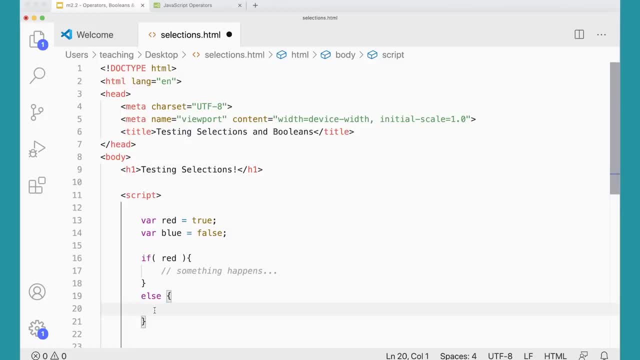 And then something else would happen here: Consolelog. the statement is false And up here we'll do consolelog. The statement is true. Very exciting. Now we can try this out And come over here to our browser. I'm going to make a new tab here. 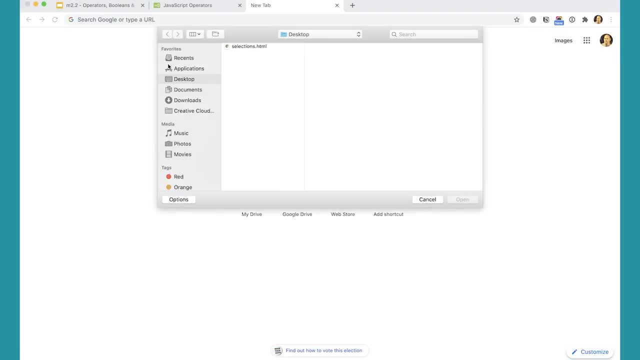 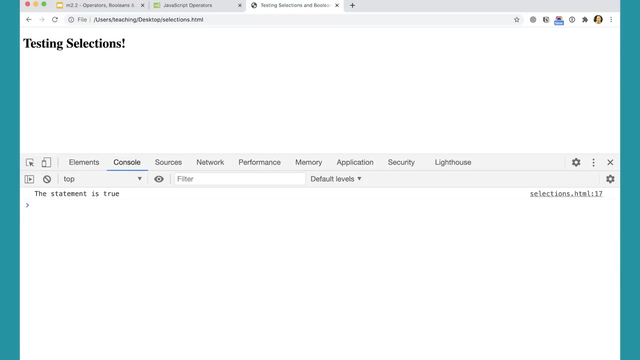 And I'm going to open this file. Selections Open And I've got my testing selections. If I right-click and choose inspect, I can go to the console And, sure enough, the statement is true. Now I can come back to my code editor. 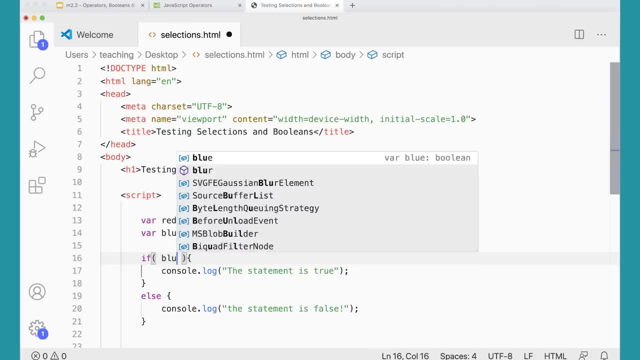 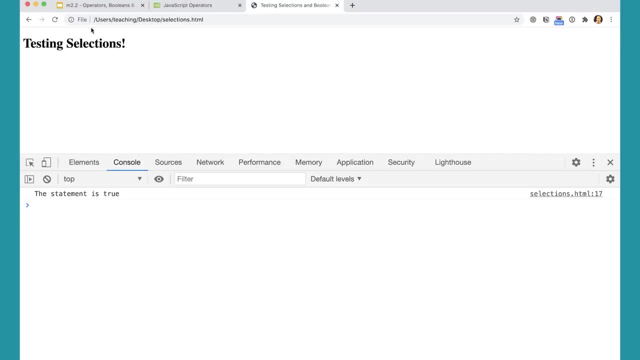 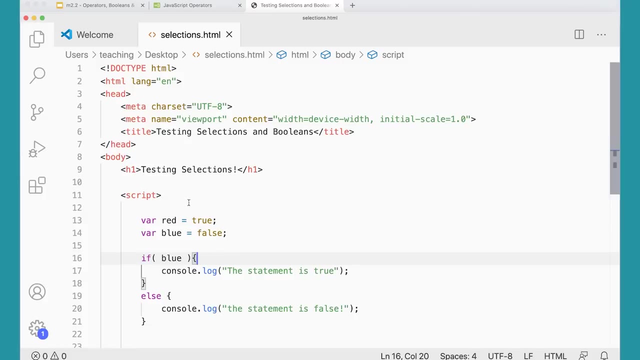 And if I change this to blue, blue is false, So this statement will run. So if I come back and then click refresh now the statement is false. Or alternatively, I could change the value here to false. Change that back to red. 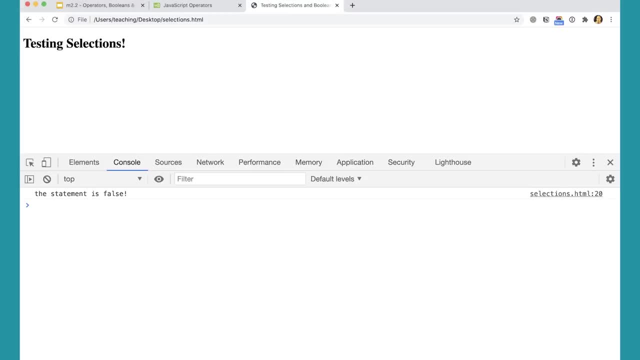 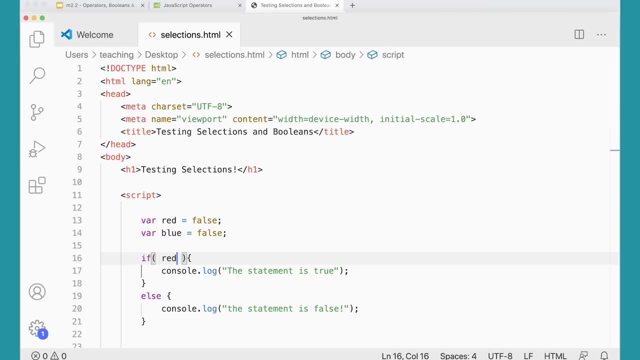 Save that And then come back and you'll see that in fact, it's still coming up false. One thing to note is I've added some extra spaces in here. Usually you won't see programmers doing that. Usually you'll see it more like this: 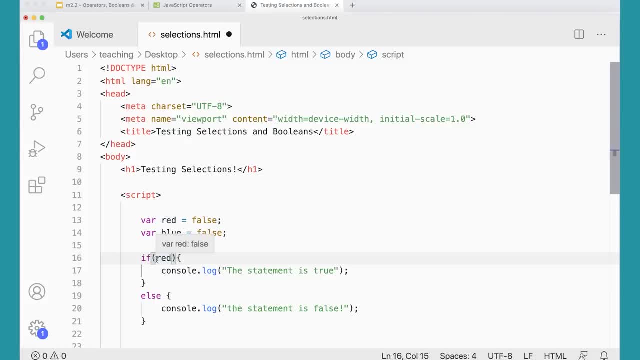 I just add the extra space in there just to make it a little bit easier to read and a little bit easier to evaluate. But the spaces aren't necessary there. Oftentimes you'll see a space here, And that's fine too, But it's not necessary either down here. 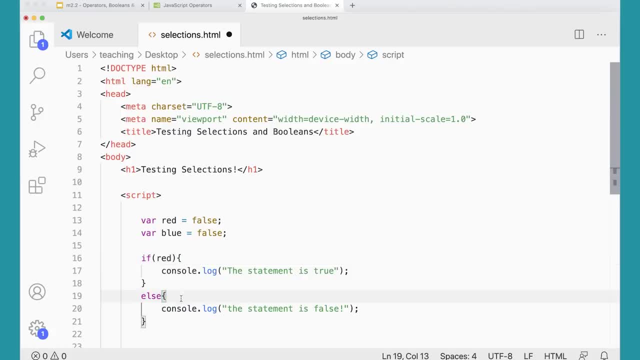 I just want to put a space in, whether I want it or not, And that's fine. So red is either false or true, And blue is either false or true because I've used these booleans here. True, The syntax highlighting should help you. 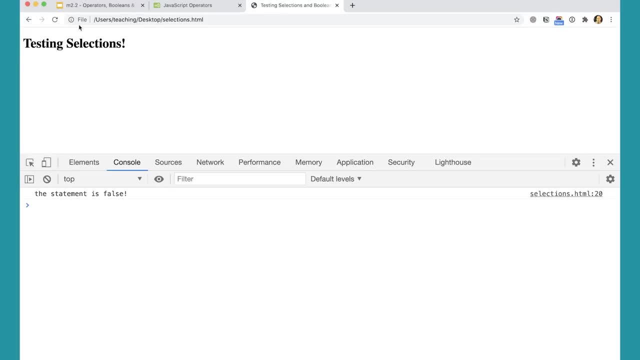 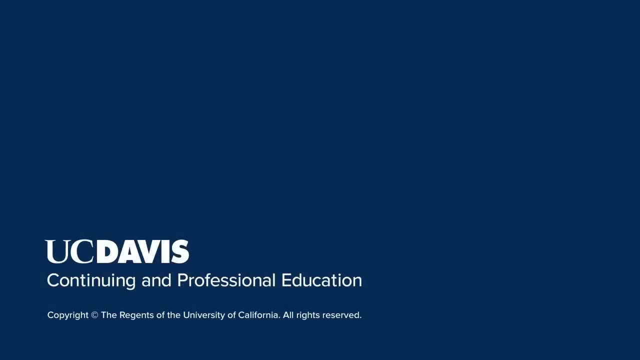 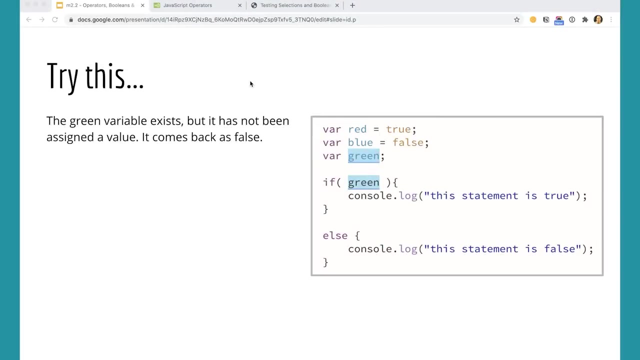 If you spell true, wrong, like I just did, it should tell you: whoops, something's wrong there because the color isn't right. And now the statement is true. This is interesting. Let's try this. I'm going to make a variable called green and then see what happens if I pass green in here. 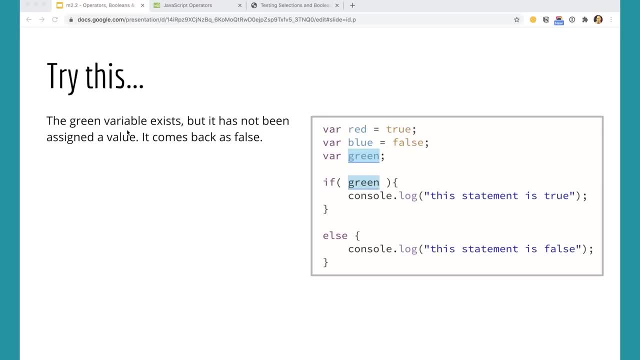 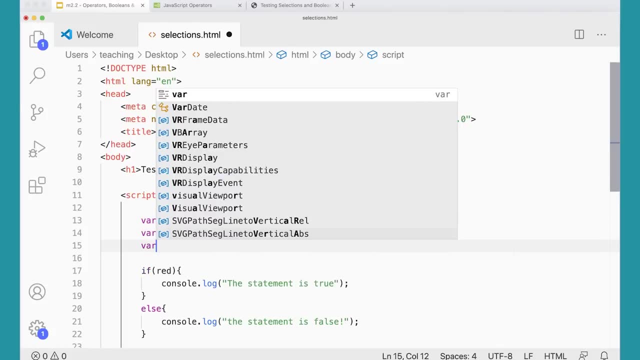 Notice, green doesn't have a value here, So let's take a look at that. I'm going to make a variable green and just put a semicolon And then down here I'm going to test: green- Is green, true or false? What do you think is going to happen here? 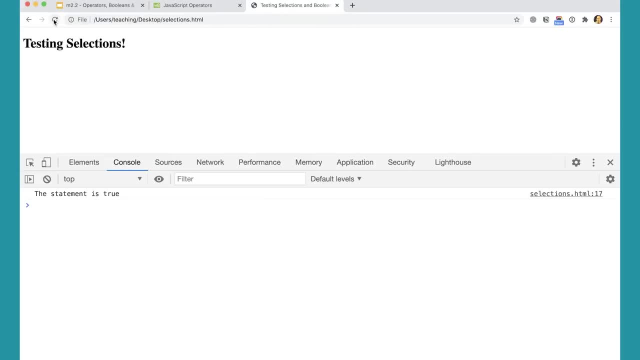 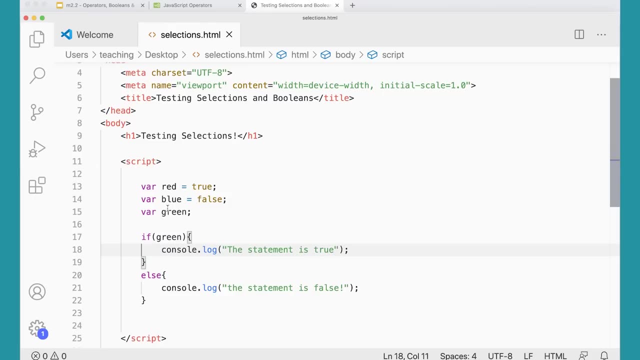 Let's test that The statement is false. This is an important thing to understand about JavaScript. Green is essentially undefined. It's an undefined variable. Undefined resolves as false in JavaScript. JavaScript has a concept of truthy and falsy, Which is kind of fascinating. 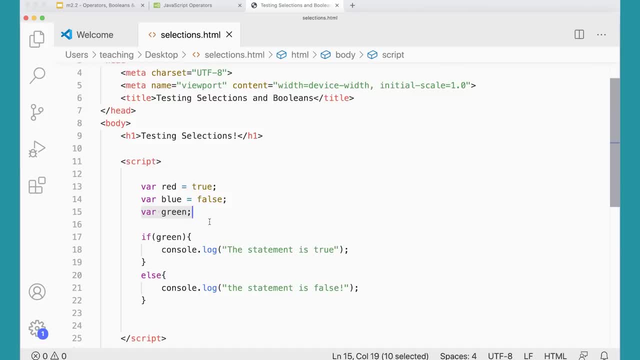 So things are either true-ish or false-ish, And they could be explicitly true or false, like red and blue are here, But they could be false-ish, And JavaScript treats variables that are undefined as false. Also, whoops, green equals null. 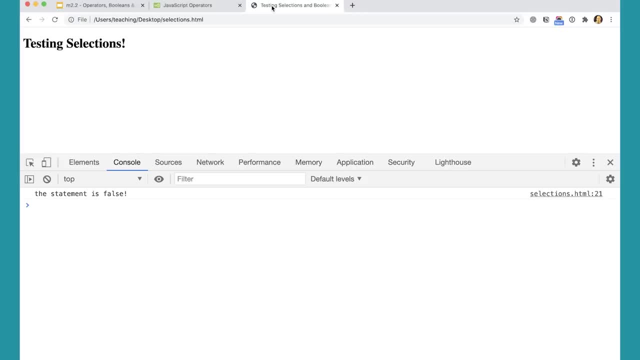 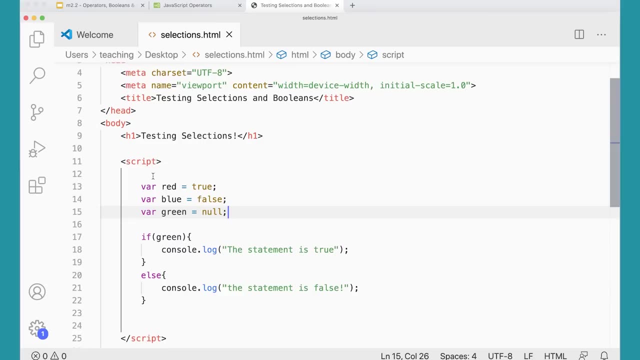 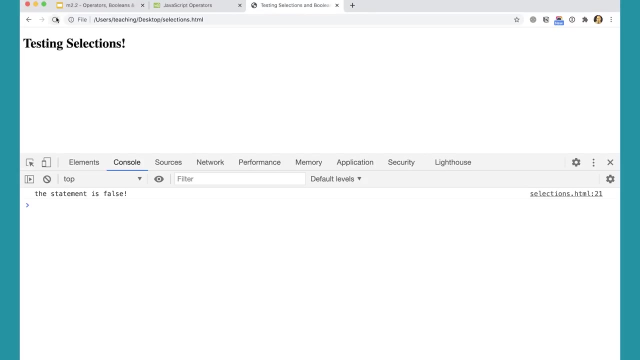 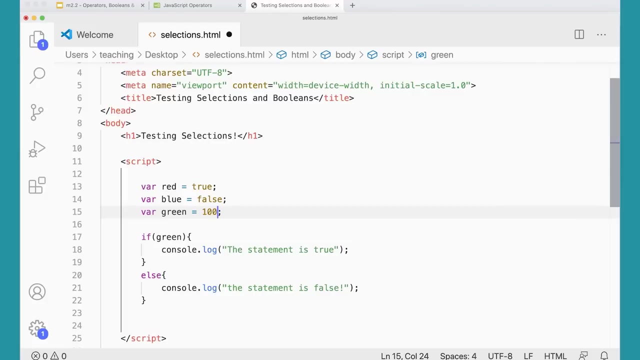 That will be false. So that comes up false. Green equals zero. Zero is false. But if I put any other number in there, any other real number like a one One is true. What about 100?? That will be true too. 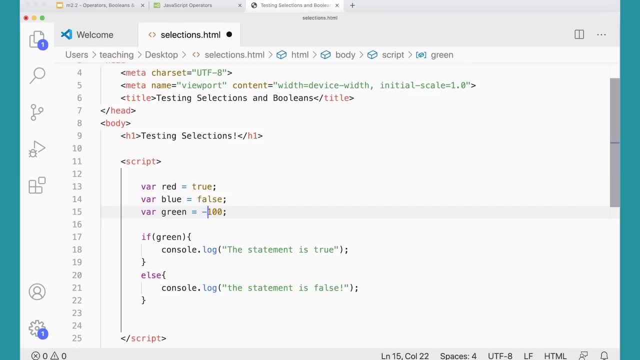 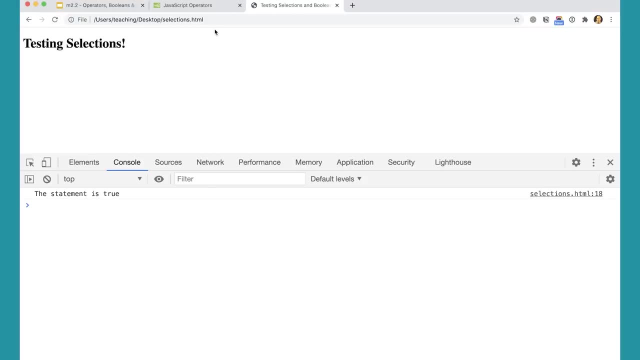 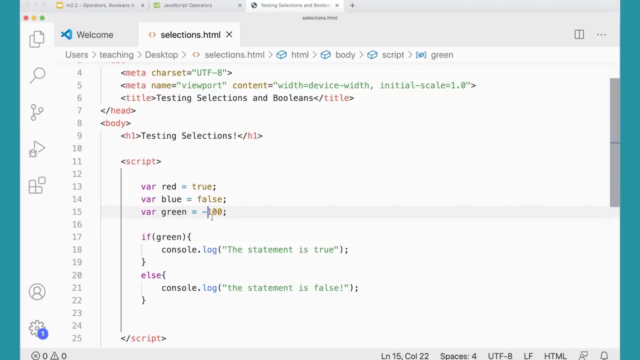 What about minus 100?? That's true as well. So numbers are true, except for zero. Zero is falsy, So zero comes up as false, Which is kind of an interesting thing. So things that we know are false are undefined as false. 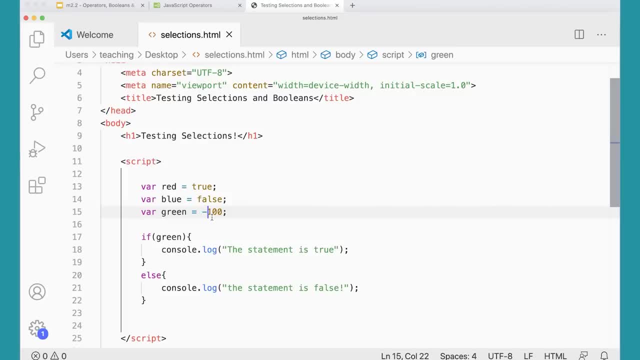 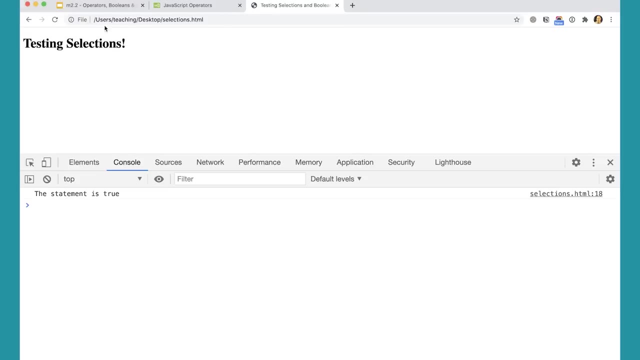 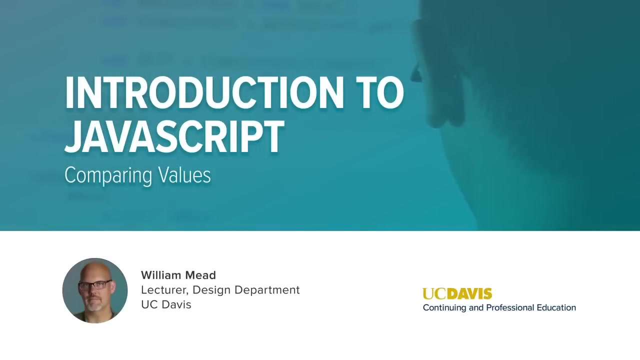 Null is false, Zero is false, False is false. Other things are true. What if I put like cheese? That's true, Cheese is true. So that's a very interesting thing about JavaScript. Let's look at comparing values. 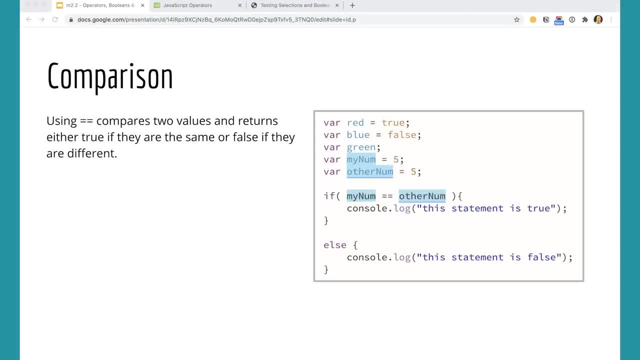 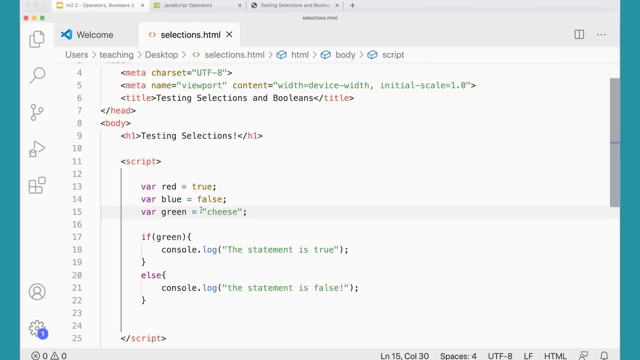 This is something we'll do a lot in JavaScript, So we often want to find out if the value here is the same as the value somewhere else. So I'm going to go back and leave green here as undefined, like so, And then I'm going to make a new variable, var mynum, and assign it the value of 5.. 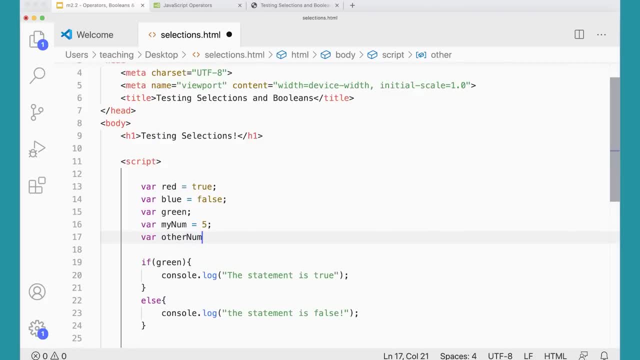 And var othernum and assign it a value of 5.. And then down here I can check to see if mynum Is the same as equals equals othernum. It's really important to read this as the same as This is assigns. 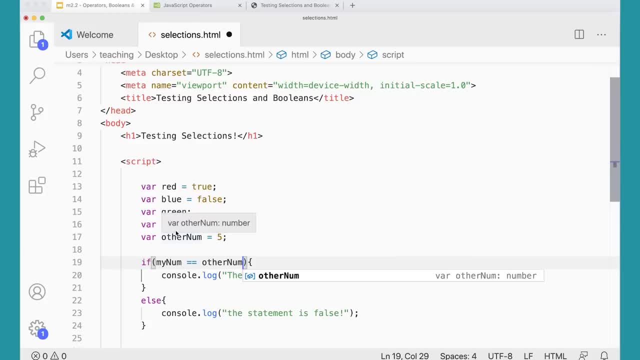 5 is assigned to othernum And 5 is assigned to mynum. But here I'm checking to see: is mynum the same as the othernum, And in this case it is. So if I save this and test this, 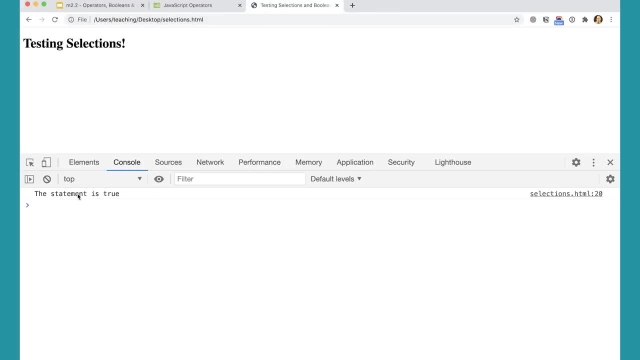 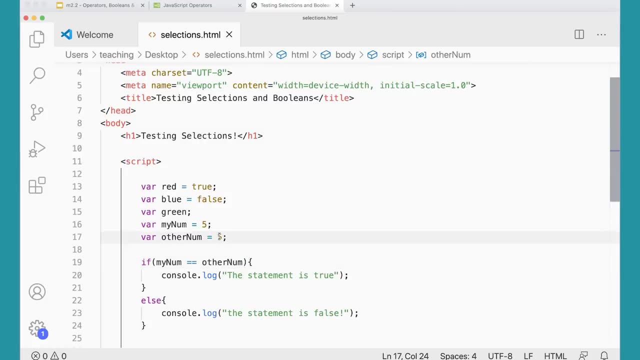 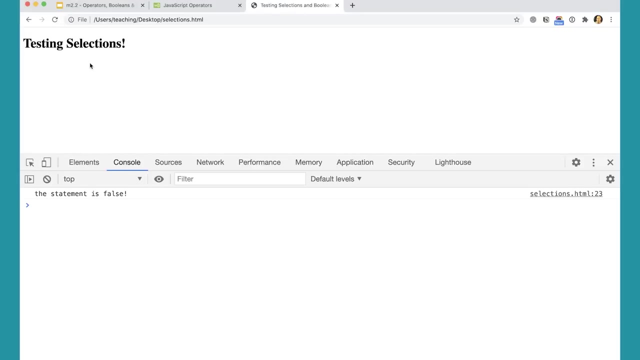 You'll see the statement is true Because mynum is the same as the othernum. Okay, If I change this to a different number, then I'm obviously going to get false. That's not true. So the statement is false. They're not the same as. 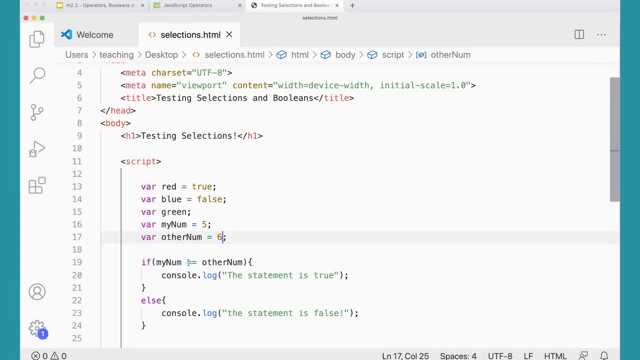 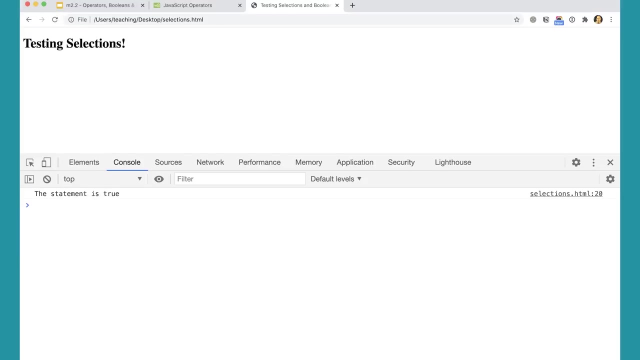 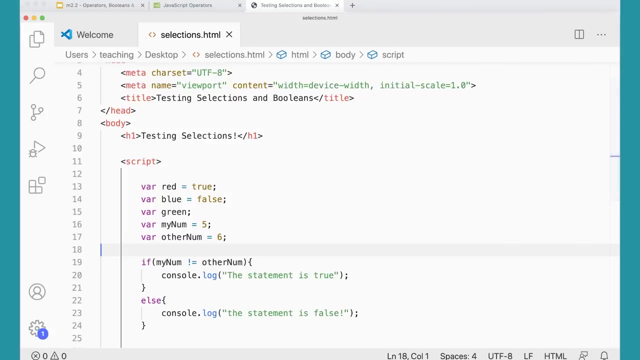 I can use, instead of equals, equals, I could use exclamation point: equals, And that'll be not the same as So is that true? Is mynum not the same as othernum? Yes, that's true. Statement is true, So we can do this kind of thing as well. 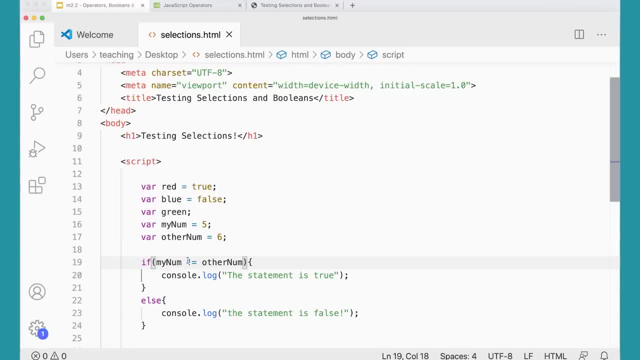 We can also use. we can also check for greater than or less than. So we could say: is mynum Less than Oops? Is it less than My othernum? And that should be true, Because mynum is less than the othernum. 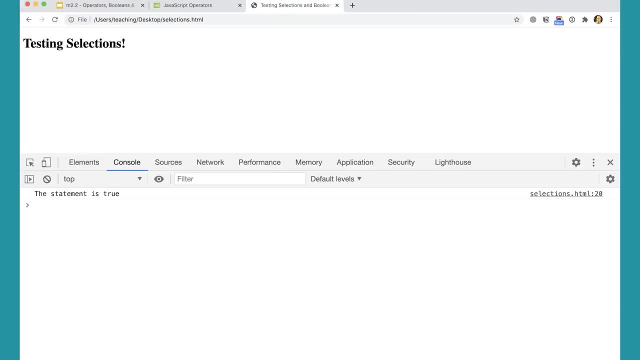 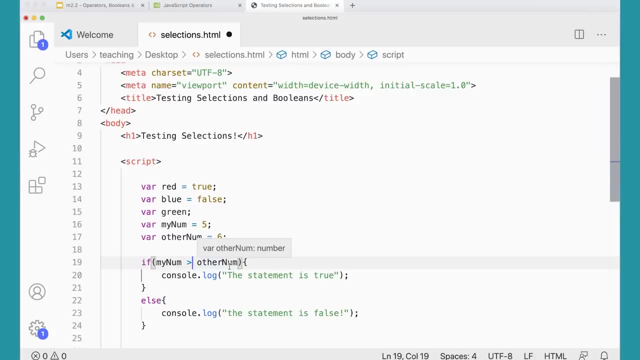 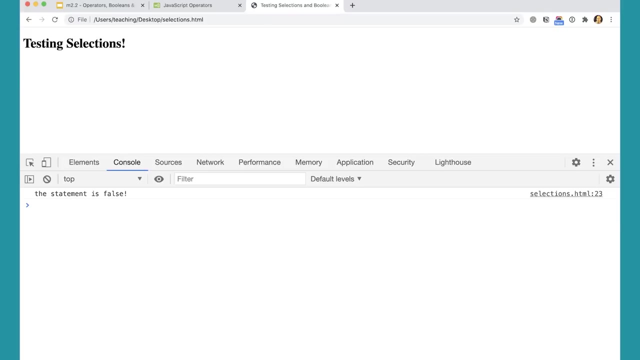 Let's see. And that statement is true, I could put: Why is it greater than? Is mynum greater than the othernum? Is that true? That's not going to be true, Because five is not greater than six, But we can test for these different kinds of scenarios. 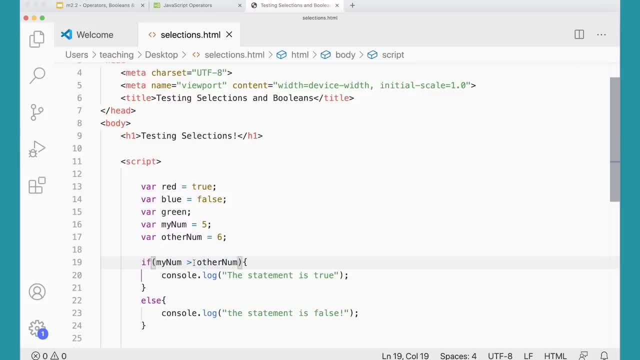 Mynum and othernum. We can use less than and greater than And check to see if that's true. Let's try this out. This is interesting. var not num equals quote five, So this five is a string with the number five in it. 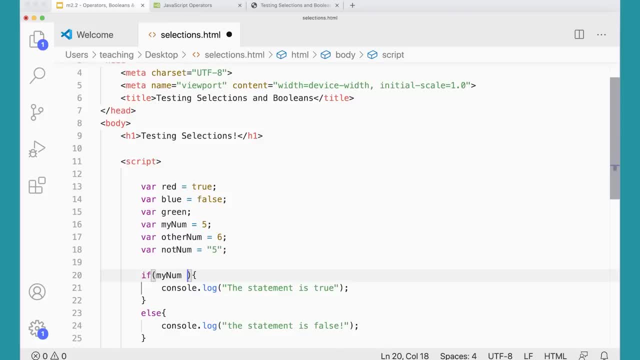 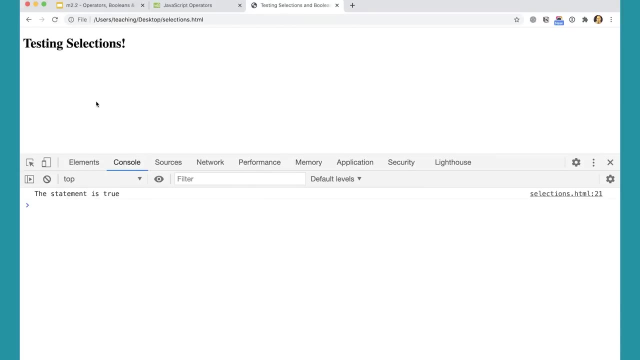 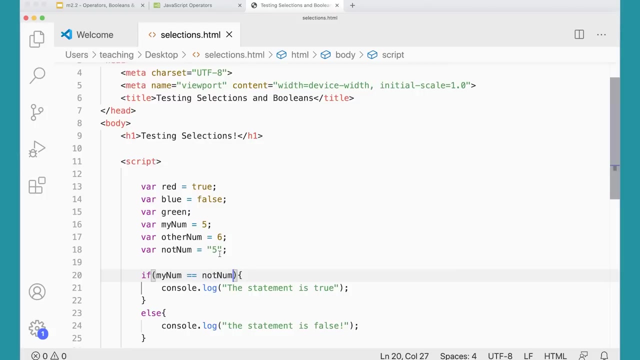 Now can I check to see if mynum is the same as not num? What do you think I'm going to get there if I save that and try that? The statement is true. Well, that's interesting. How can a five be the same as five inside quotes? 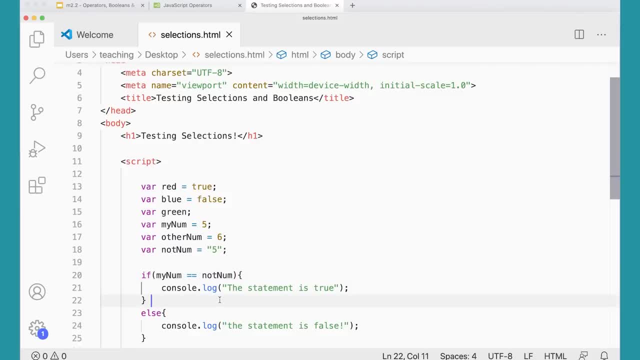 Remember, JavaScript is loosely typed And it allows for something called type coercion. So what's going on here is that JavaScript is saying: well, we've got a five here And we've got a five in a string, And they're basically the same. 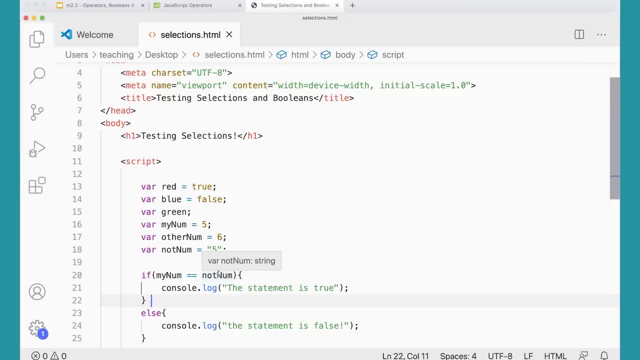 So I'm going to call that true. So that's truthy, You know, it's true-ish sort of You can think of it that way, Which is very interesting. Now, again, this is the kind of thing that can drive programmers crazy. 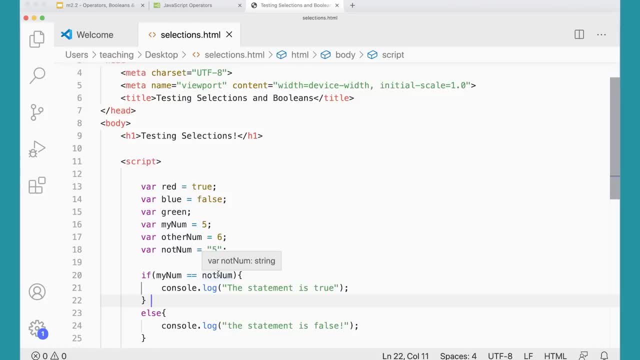 Because you could end up making a mistake in your program or having something unexpected happen, And you don't want unexpected things to happen in your program, So it's never a good thing. So with I believe it was ES5 in 2009, they introduced the triple equals operator. 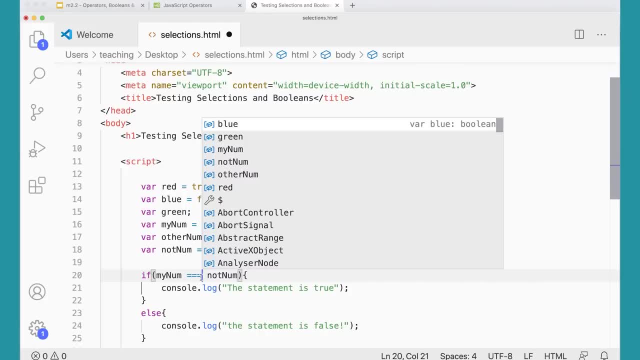 Which is exactly the same as, And that won't do type coercion. And remember, this is the kind of thing that we're working with in JavaScript. They don't want to just get rid of the double equals or change what it does, Because that would break other programs. 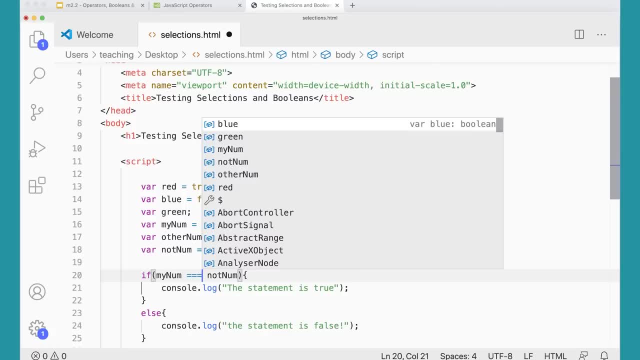 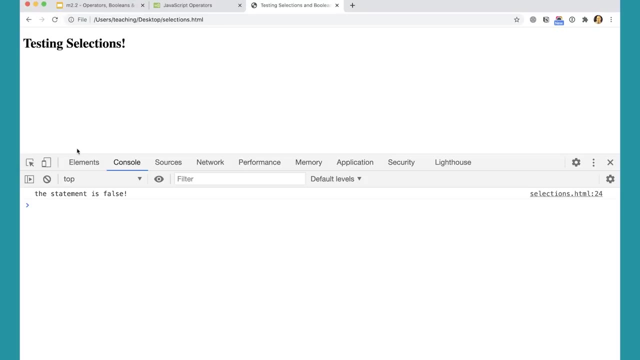 That would break programs That have been happening in the past. But they can add another operator, Which is the triple equals, And that one will not do the type coercion. So you'll notice this one will come up false. That statement is false. 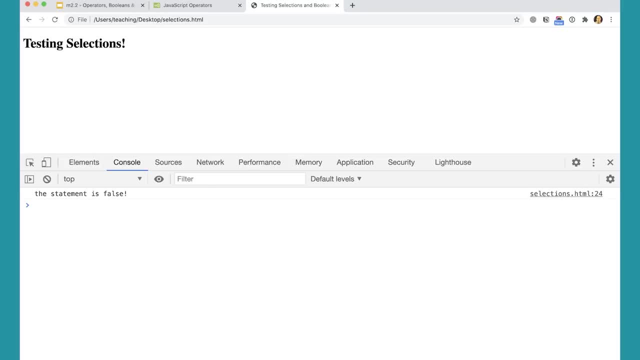 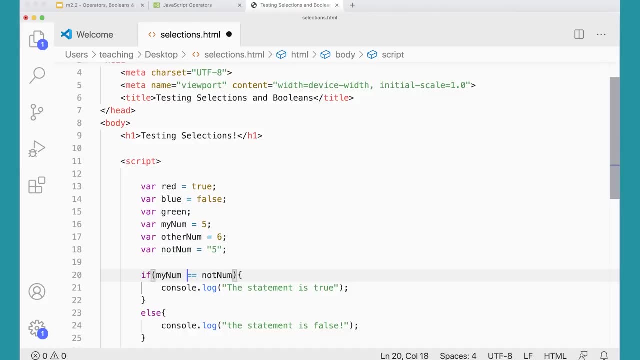 Because it won't do the type coercion. There's also the same thing with the exclamation point, So you could say that's not exactly the same as. So you can read this: as is my num exactly the same as not num? And the answer is no. 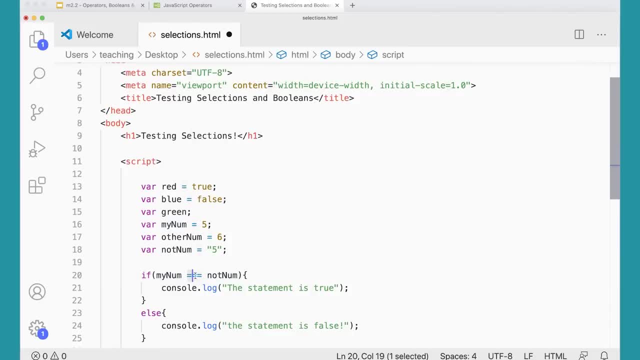 Generally it's considered better programming to use the triple equals sign everywhere. Often in our shorter scripts it doesn't really matter And you'll see me use equals, equals all the time. But really, you know, if you want to get in the habit, get into really good habits, always use the triple equals sign. 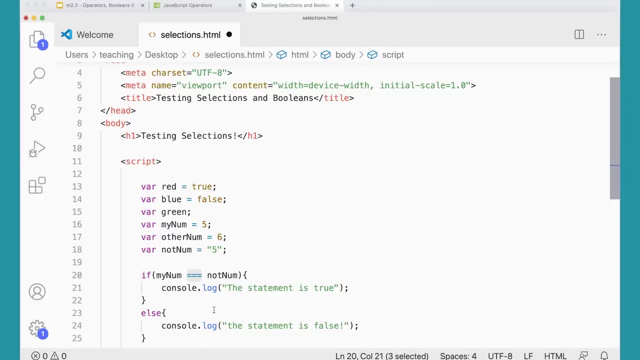 So that you don't ever have any type coercion, Unless you really want it for some reason. And again, this is kind of an odd thing about JavaScript that it can do this, But it makes the language very expressive And that's kind of interesting. 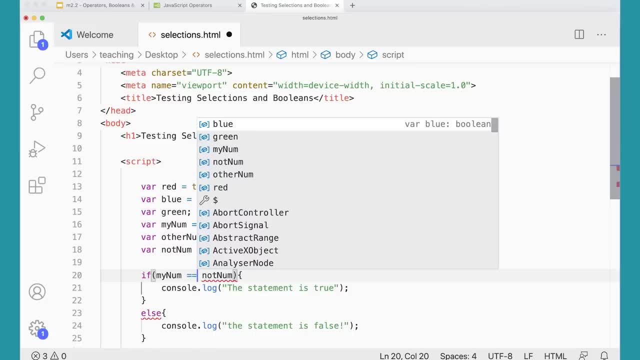 Expressive in the sense that, you know, these things are kind of the same. A number five is the same as the five in quotes, So that's kind of interesting. One more thing I want to check out here really quickly while we're here. 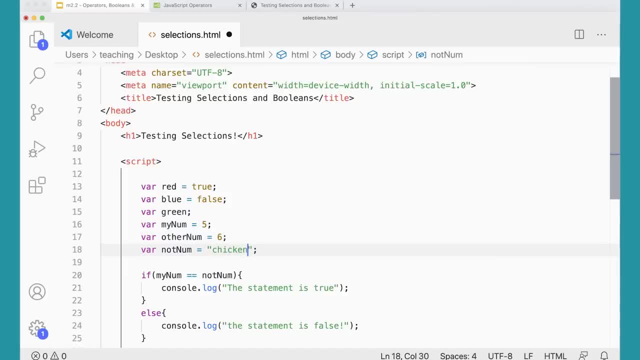 I'm going to change this five to something like chicken And then I'm going to make a new variable, Var. my value equals, not num minus my num. What the what? I'm going to take a chicken And subtract five. That doesn't make any sense. 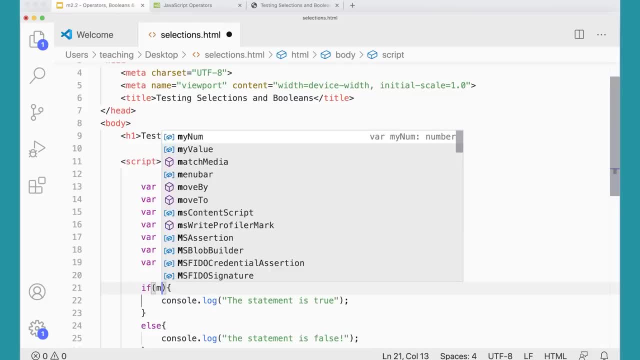 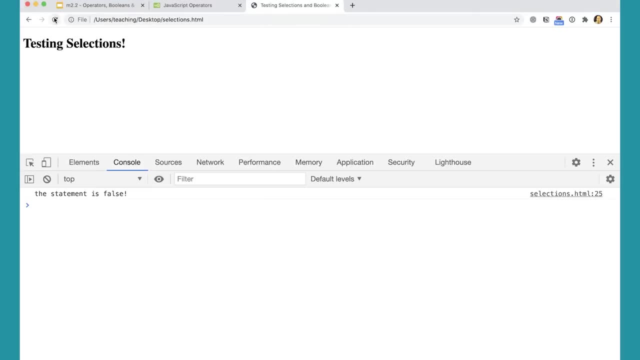 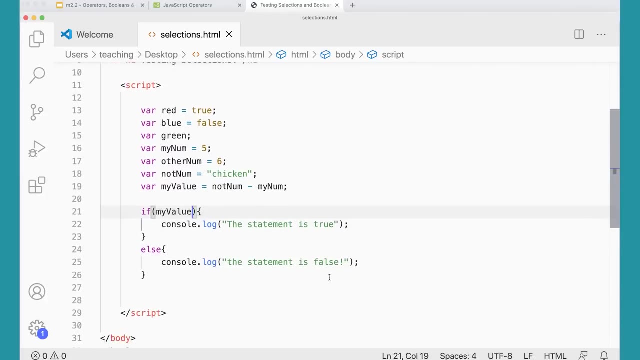 What happens if I put my value in there? You probably won't be surprised to see that that comes up False, That's false, And more than that. if I come down here and just consolelog my value Just to see what's actually in that value, 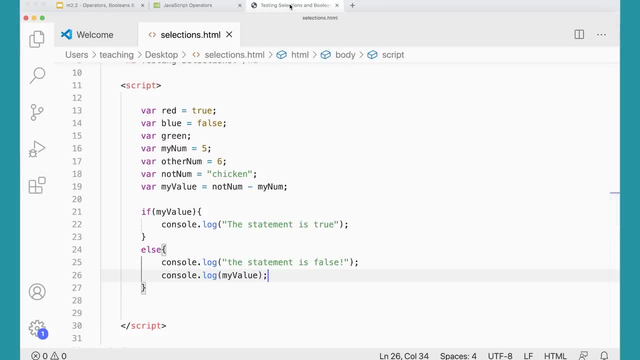 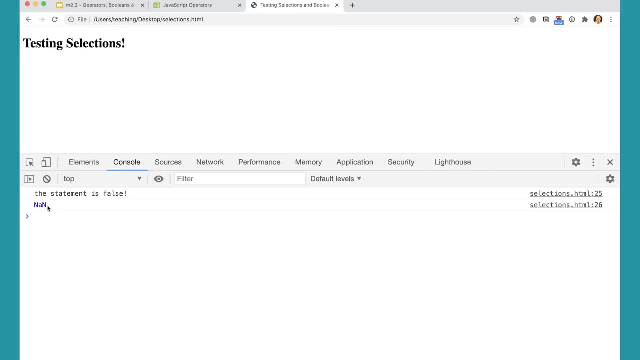 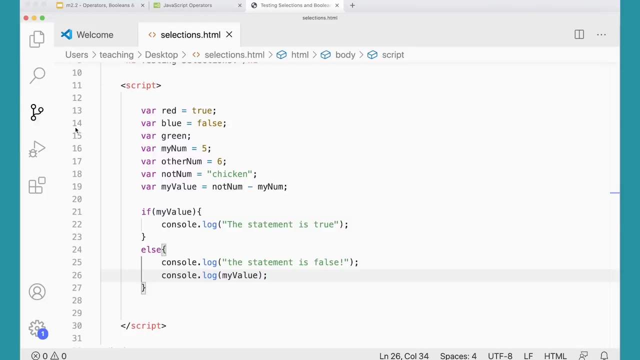 My value. When I try to take a chicken and subtract five from it, What do I get over here? Nan, Not a number. Nan is another thing in JavaScript that is falsy. So in our list of things that are false are zero. 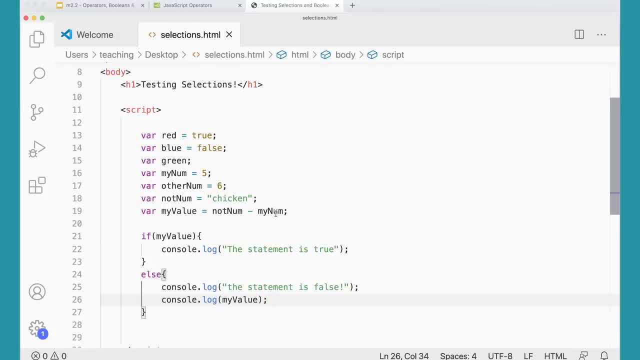 False, Undefined Null And not a number- Those things all come up false in JavaScript And that's kind of an important thing to keep in mind as we move forward with working with JavaScript and working with Booleans and when we're testing values. 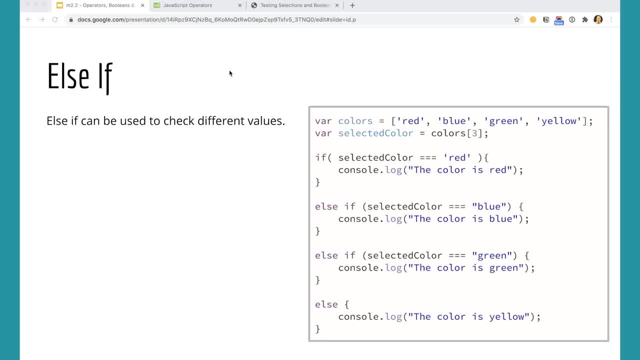 JavaScript has an else. if So, we can run through a series of selection checkers to see which one is true. So let's type this out. It's always a good idea to practice this stuff as much as you can and get used to the syntax. 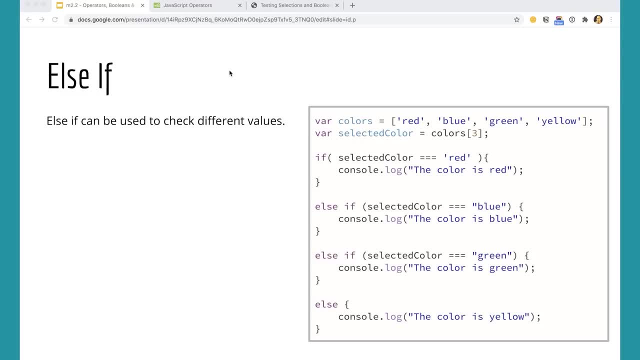 Again, there are two hunks to get over with JavaScript, And the first one is done just by practicing, by just writing the stuff and making mistakes and forgetting to put in the semicolon or the curly braces or the square brackets, and seeing what happens when you get an error. 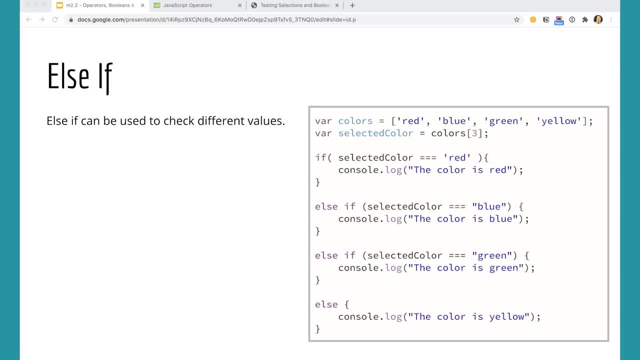 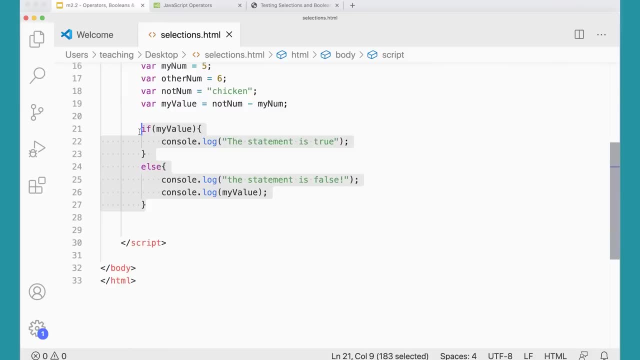 So let's go ahead And type this in over here. So I'm going to come back here and I'm going to add: you know, maybe I want to comment this out In Visual Studio Code I can do Option, or in Windows Alt-Shift-A, and that will put a comment around something that I've selected. 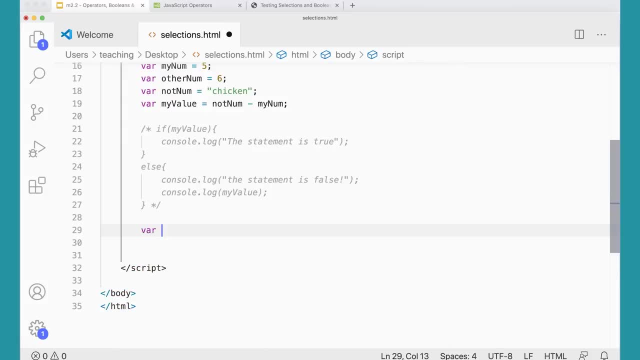 So down here I'm going to make a variable Far colors equals square bracket. Quote: Red, Green, Blue, Yellow. I'm going to make a variable var- selected color Equals colors Square bracket, And we'll do three. 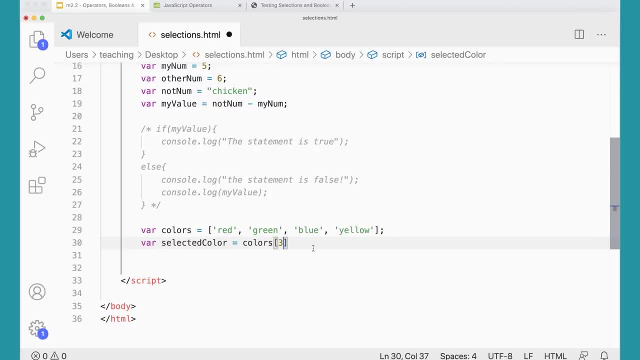 Red is 0,, 1,, 2,, 3.. Now over here. So I've got that And that's great. Now I can do an if-else statement. So I could do if Selected color Is the same as equals, equals. 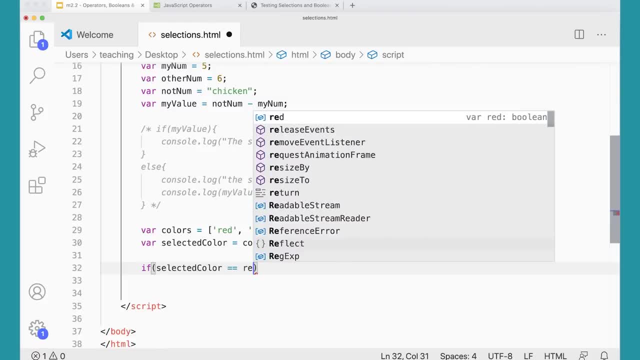 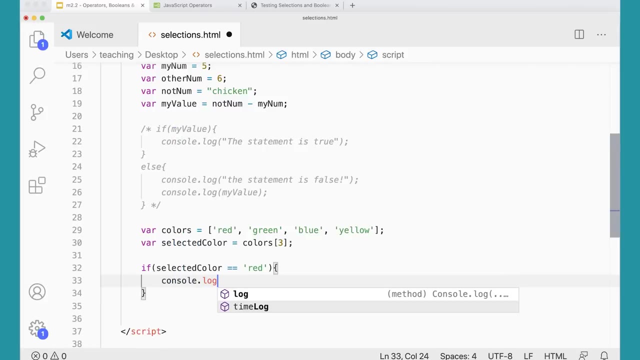 Red Or Yeah, let's do red, Red in quotes, Red. If it's the same as red, Then I can console log something out, Console dot log. The color is red. Now I can do an else if, And again I can put else if on this line here, like so: 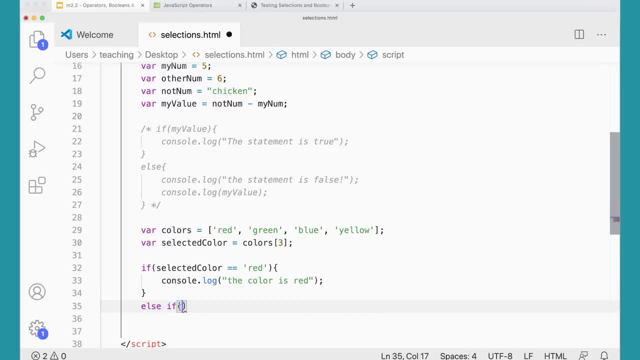 I think it's a little bit easier to read if you move it down like this: Else if Selected color. And here I'm going to cheat by copying and pasting: Else if Selected color is blue. And again, I'm just adding these extra spaces because I think it's a little bit easier to read. 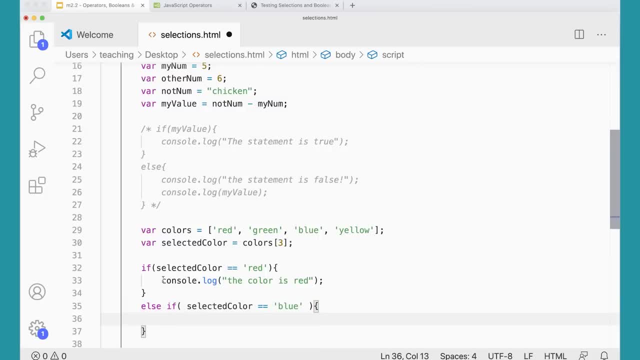 But it's not really common practice. But that's okay. If the selected color is blue, then I'm going to console log out Blue, Actually I should do green. Green is next, It doesn't matter, I can go whichever order I want. 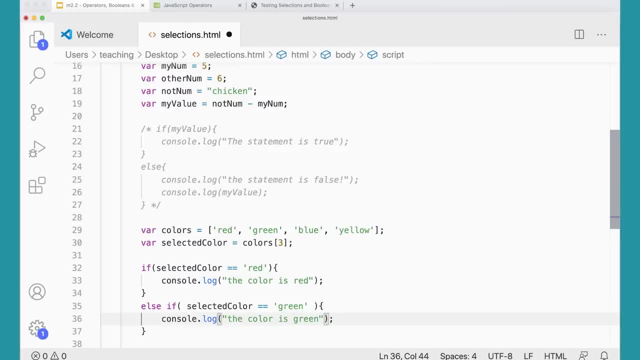 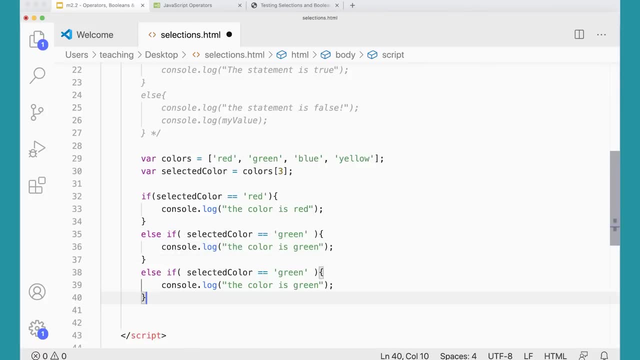 In this one I'm just going to go to green because that sort of makes sense, And then I can copy and paste the else: if Selected color is, Change this one to blue, Blue, And if it's not red, green or blue, then it must be yellow. 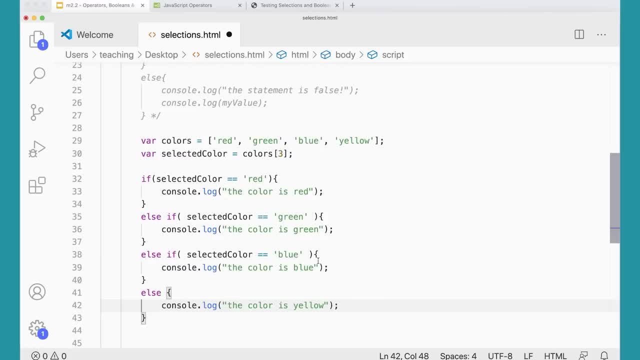 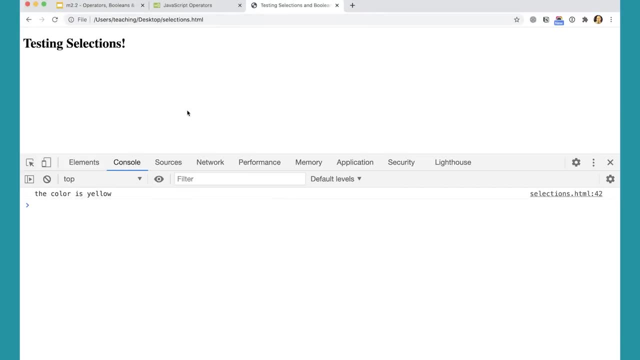 Okay, Great. So with this script in place, we can test this. We can come over here And refresh. Refresh this And you can see the color is yellow. It went through that list of items and chose the correct color. 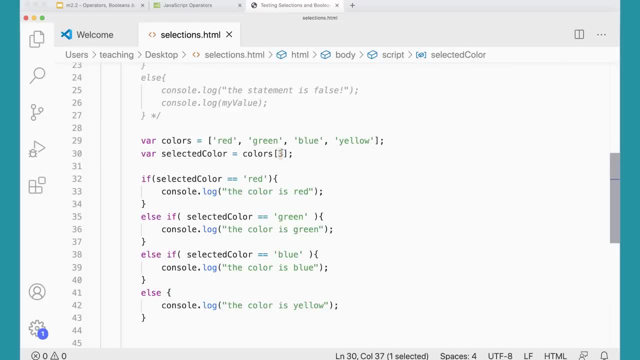 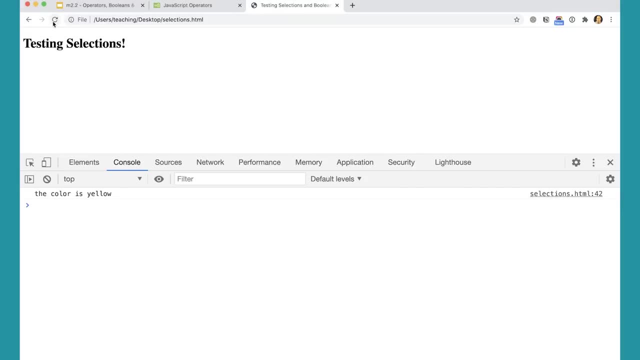 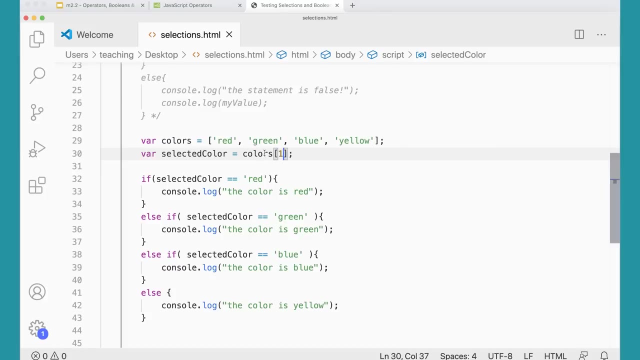 Whereas if I come up here and change this to a one, So zero one, And I run this, You'll see I get. the color is green. Now what happens if I make a mistake? Suppose I put four Zero one. 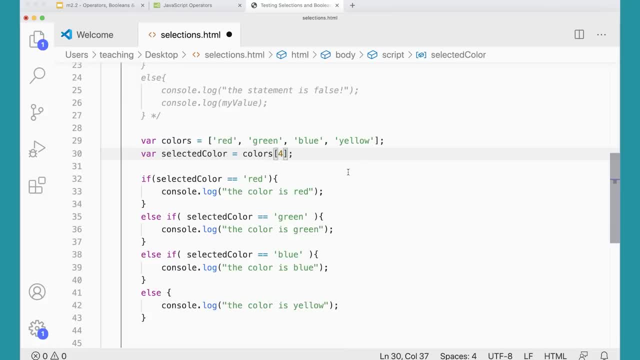 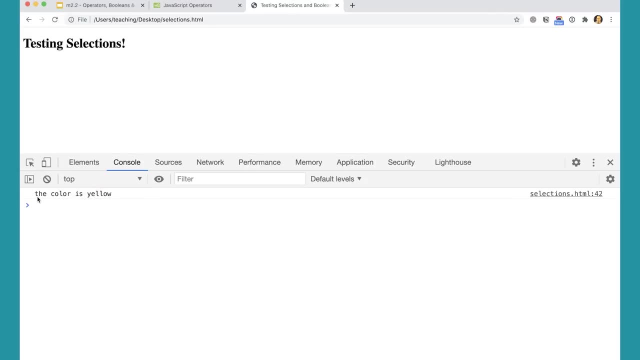 Two, three, Oops, There's no four. Let's see what I get over here. You're going to get mistakes, You're going to have errors And, this said, the color is yellow because the else ran, Which is not really what I wanted. 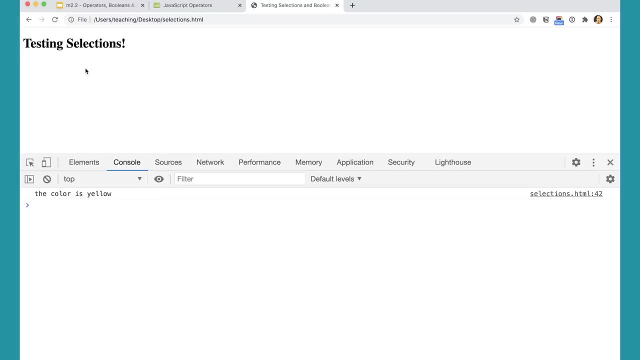 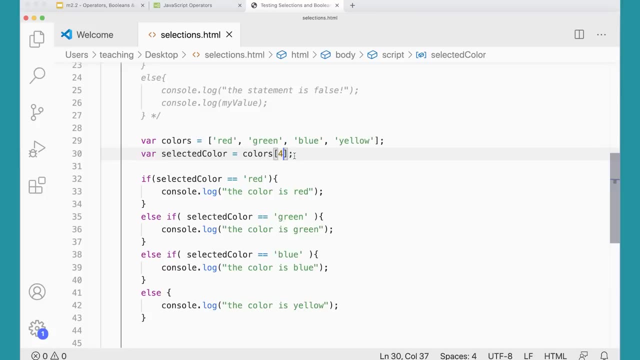 But it is sort of doing that kind of thing. Or let's see what happens if we do. What happens if I make a mistake And I forget to put commas in here? This is a common mistake that I see from students Is they'll forget to put the commas in the array. 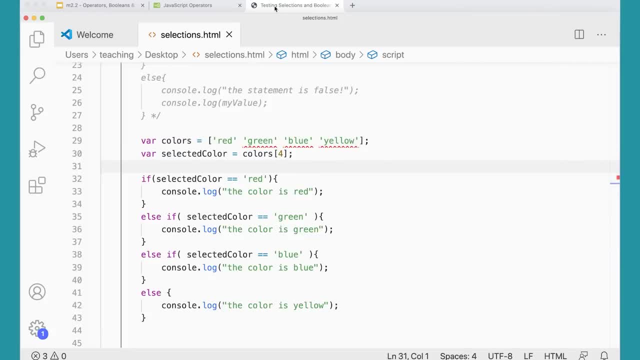 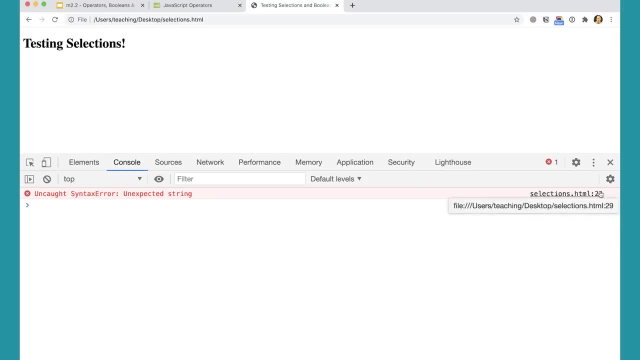 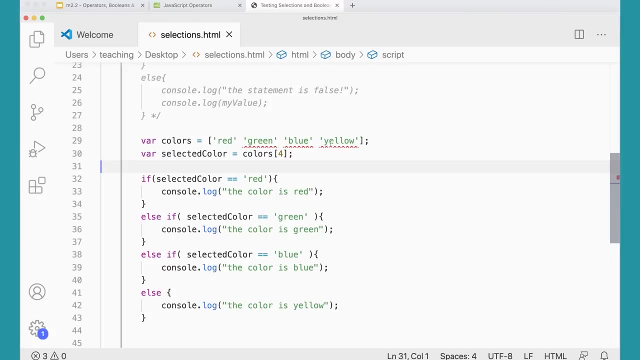 What happens if I do that? Uncut syntax error: Unexpected string on line 29.. So that gives you a notion that you should come back and take a look at line 29. And see what's going on in there And hopefully you know with this stuff in here. 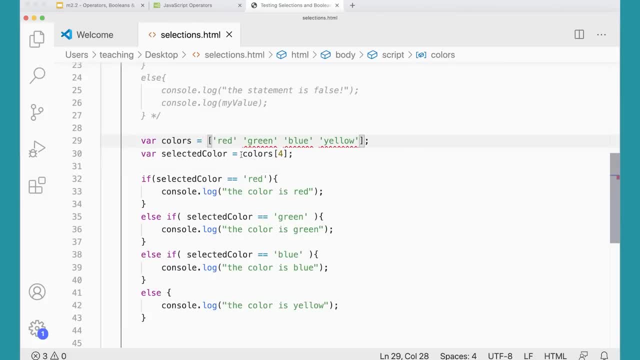 This little red underlying stuff going on in here. You'll see that something's wrong there And you'll put the commas back in- Very common mistake when you're starting with this thing. Okay, So you can try these different scripts and see how they work and what they do. 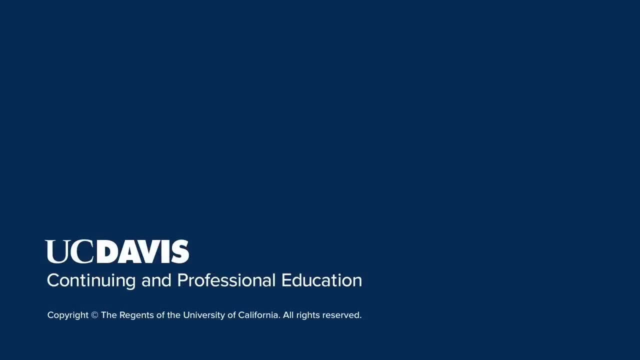 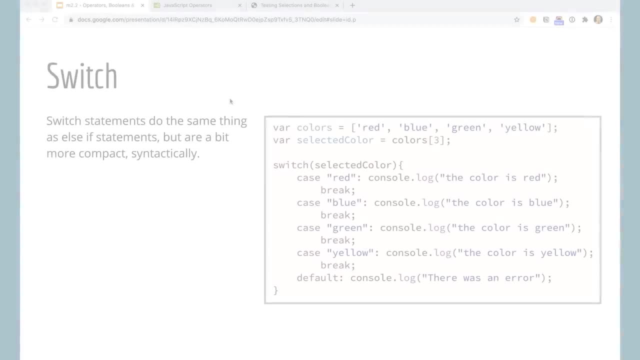 It's really helpful to do that. JavaScript also has a switch statement Which will take a value Like selected color And run it through a bunch of cases. In case it's red, it'll do this. In case it's blue, it'll do that. 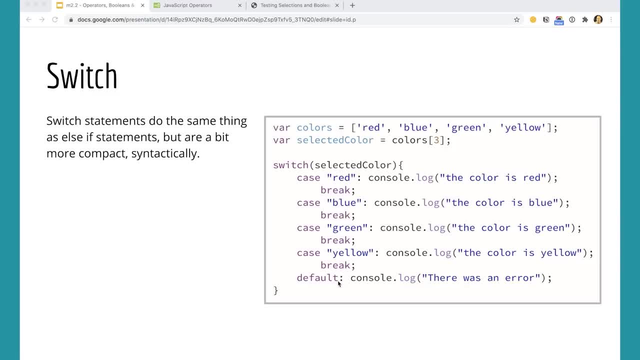 In case it's green, it'll do that, And then at the bottom there's a default. You can add a default And it'll do this if none of these other ones are true. It's important with selection That you add this break in here as well. 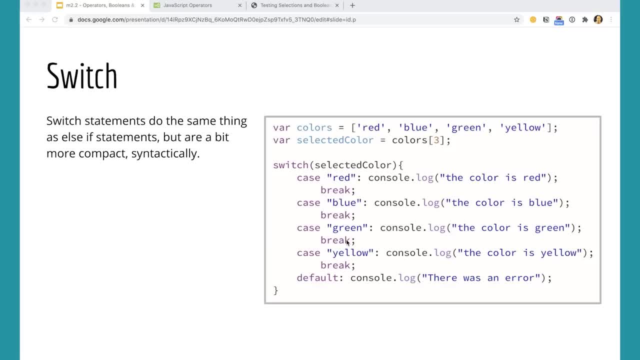 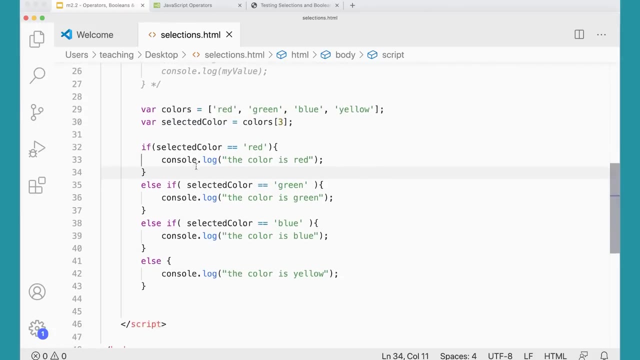 So the break will keep the Will bump out of the switch when one of these true statements comes up. So let's take a look at this really quickly And see what we get over here. So I'm going to go in here. 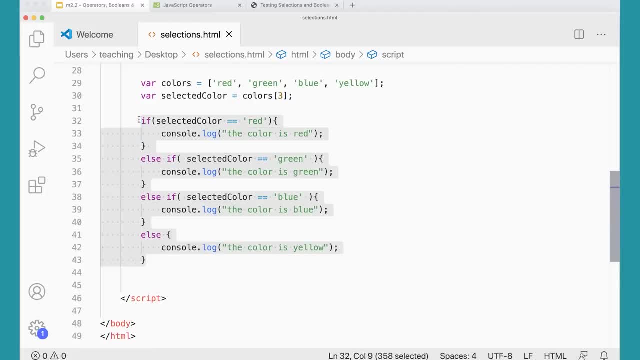 I'm going to comment out these, if else statements Again, I'm going to select them And then do option or alt shift A In Visual Studio Code to quickly just comment those out. So I'm not running that anymore, And then down here we can run a switch statement. 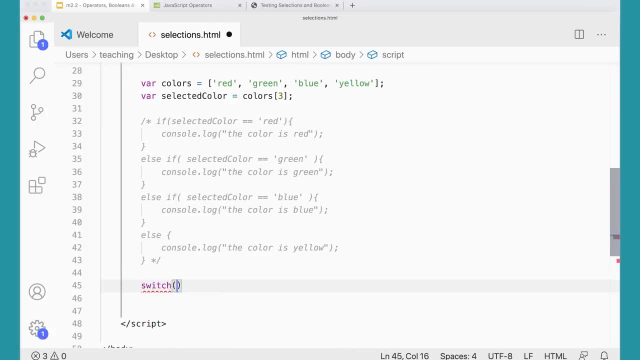 Switch Parentheses And I'm going to put in here the value I'm checking is selected color- And then the switch statement. I'm just going to paste it in here Because it's a little bit tedious to watch me type it all. 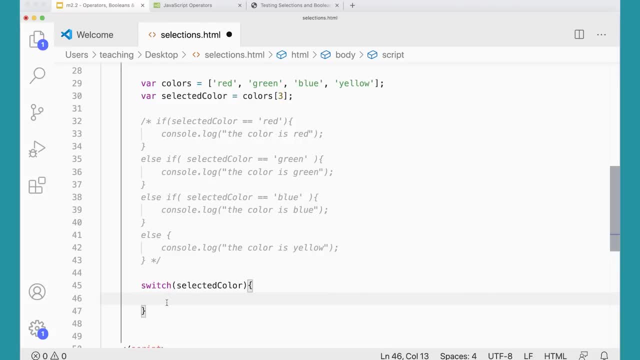 But I'm going to paste it in here, But I recommend that you type it. So type out case: red colon consolelog. the color is red And then a semicolon. So that's the statement that's going to run And then break. 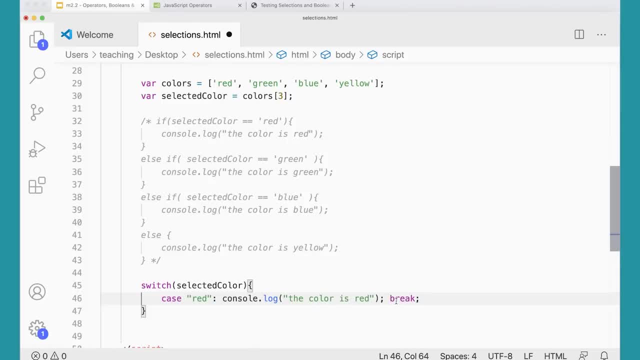 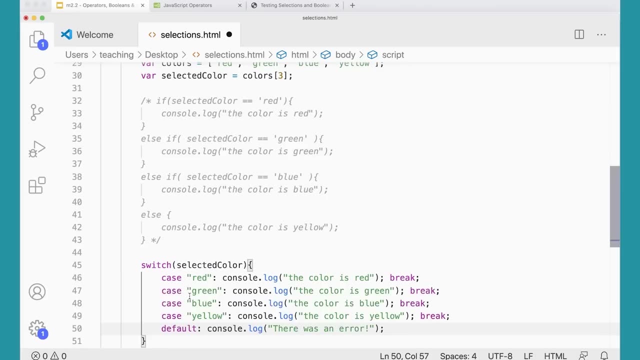 And it can be on the same line. on my slide I have it on the next line, But you can put it on the same line here. Rather than watch me type all of these, I'm going to just paste them in here, But you should type it in. 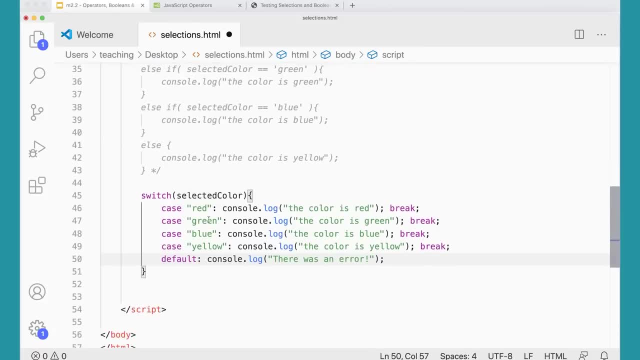 Because learning the syntax, you'll learn it by typing it, Not by watching me do it. So go ahead and make these files and type these in here so you can test it out And then notice: I've got red, green, blue and yellow. 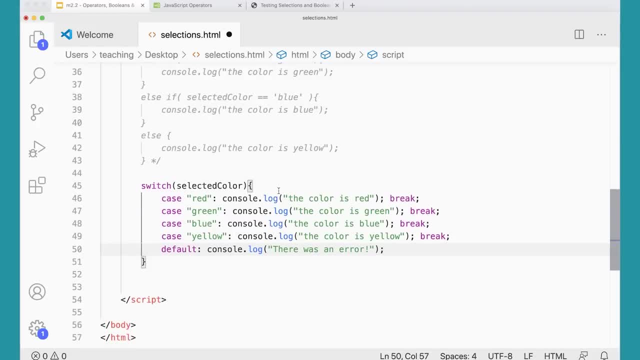 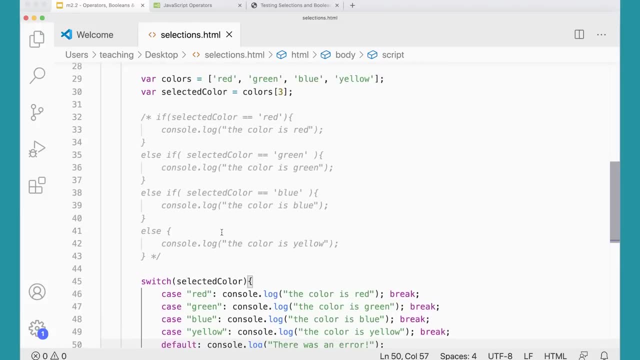 And up here. if I set selected color to 3,, I should get you know 0,, 1,, 2,, 3.. I should get yellow. So let's see if I get that. if I come over here and test this. 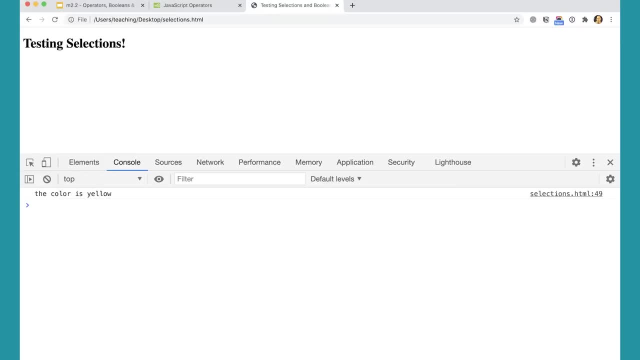 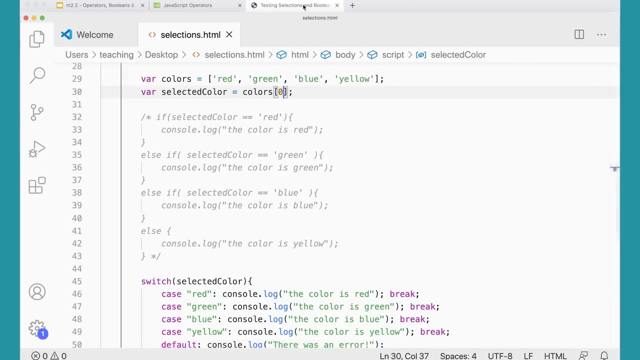 And, sure enough, the color is yellow. So that's coming up great. And I could change this to 0, which will get me the first one. So now I've got red And that break is bumping me out of there. 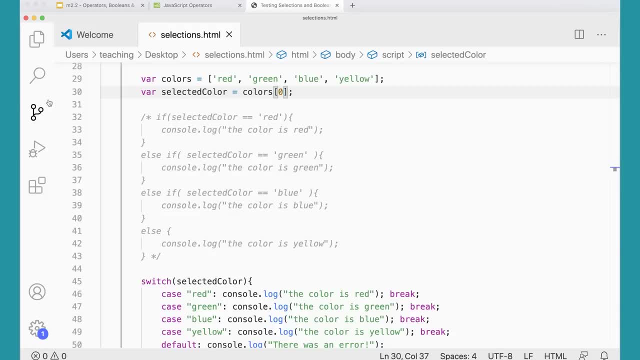 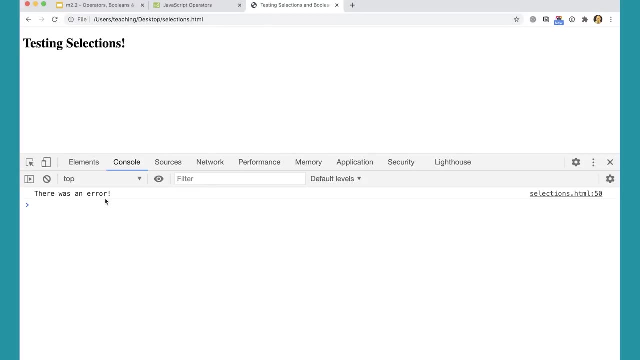 But if I were to set it to something past the end of my array? So 0, 1,, 2, 3.. If I set it to 4, the default will run And I get there was an error because I'm outside of my array. 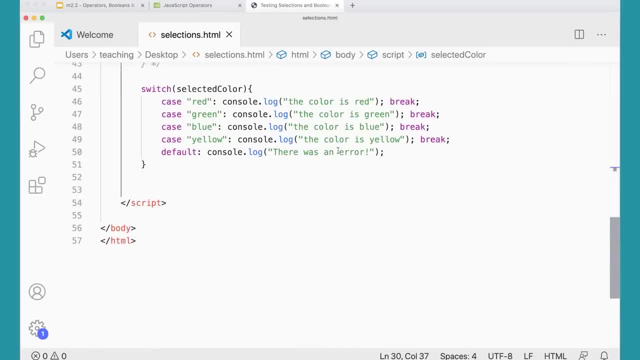 So the default option ran down here. I didn't actually create a JavaScript error. I could do that really easily by doing something like: I don't know spell break, wrong Break, And it even looks different in my code because it's not the right color. 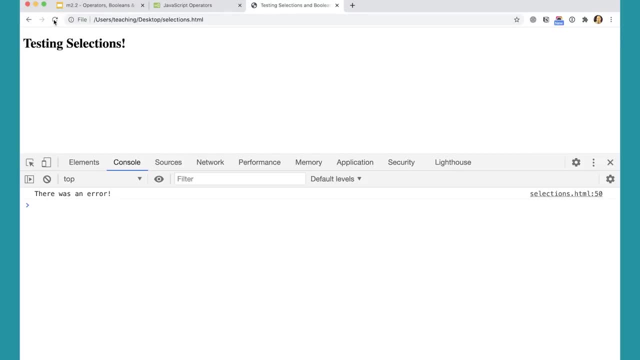 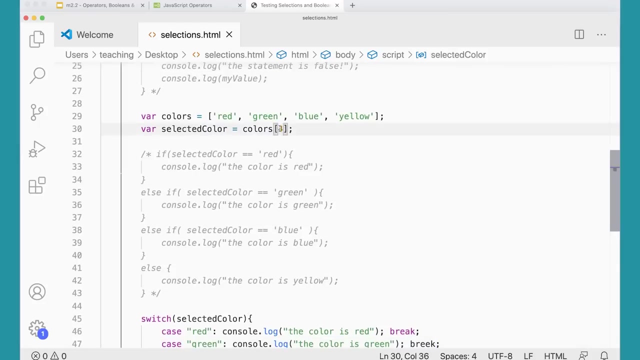 So I could do that. See what that does. Oh, it's still running. It's an error Because it didn't actually run that line, because that line wasn't true. If I set this up here to a 1, I think I'll get an error. 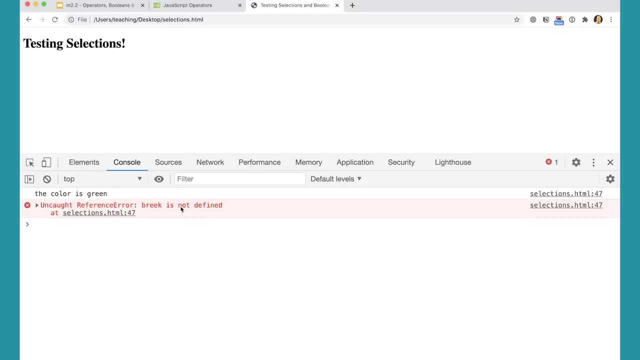 Okay, Uncut reference Error Break is not defined in line 47.. It did get the colors green, So it got that far in the script And then it ran into a problem because I misspelled that, And I misspell things all the time. 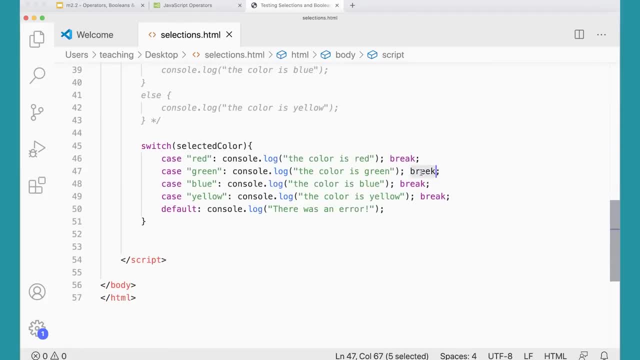 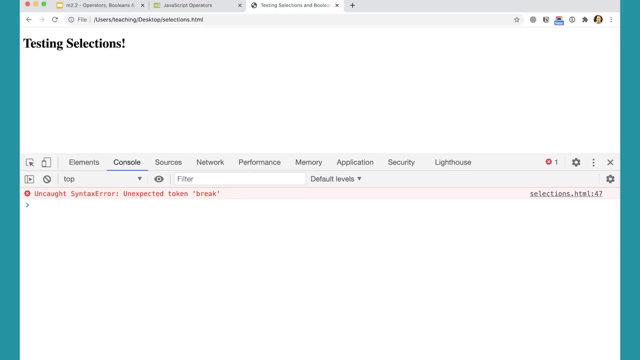 You will too. Don't worry about it, It happens all the time. Break, Or what if you forget a semicolon? Sometimes forgetting a semicolon will really set it off as well. Unexpected token break on line 47.. So these syntax are unexpected token. 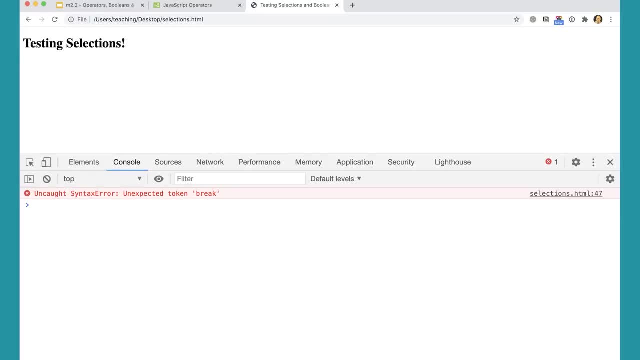 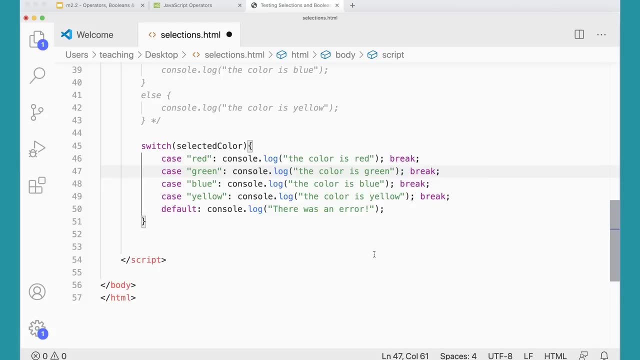 What does that mean? You know it's really expecting a semicolon token here And it's seeing break instead. So it's confused by that. But these syntax errors, these error messages, are sometimes a little bit cryptic And they take a little time to get used to them. 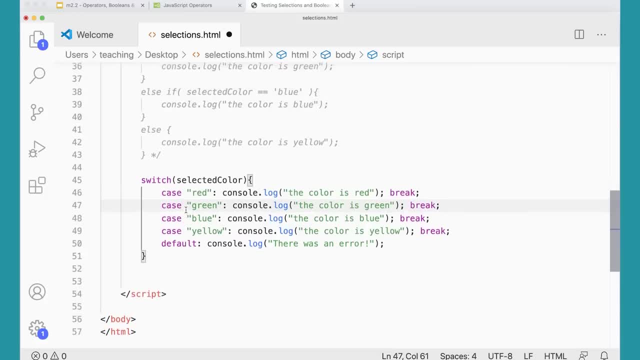 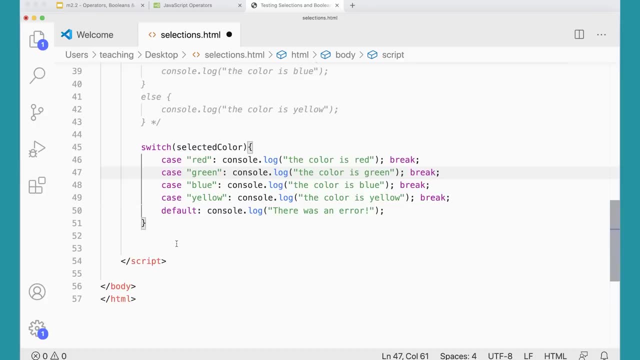 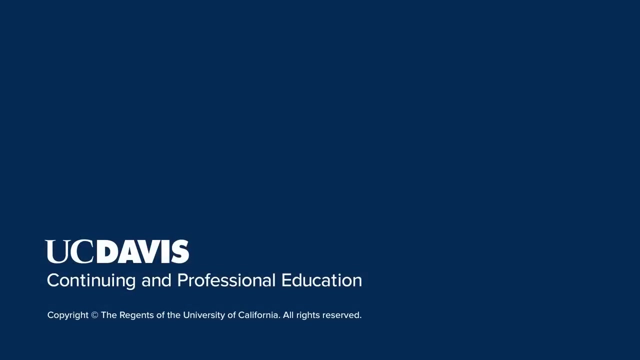 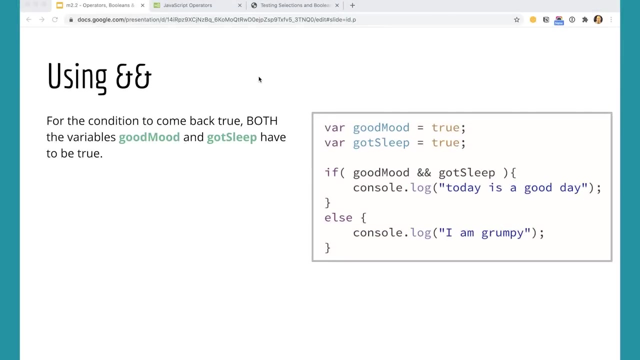 But the switch statement is a great alternative for the else if It takes up less space And it can help you be very concise and specific with your code in a way that's helpful and useful. In JavaScript, we can check to see if multiple things are true by using the ampersand operator or the pipe operator. 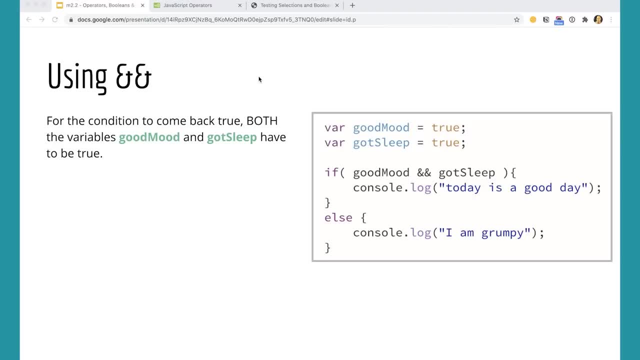 We'll look at the pipe operator next, But here we're using the ampersand operator And we use two of them together here, And what we do is we check to see if this statement is true and if this statement is true, And for this whole thing to be true, when you use the and operator, both of these must be true in order for this to run. 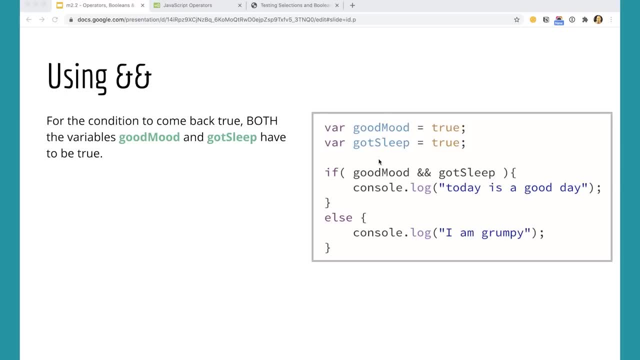 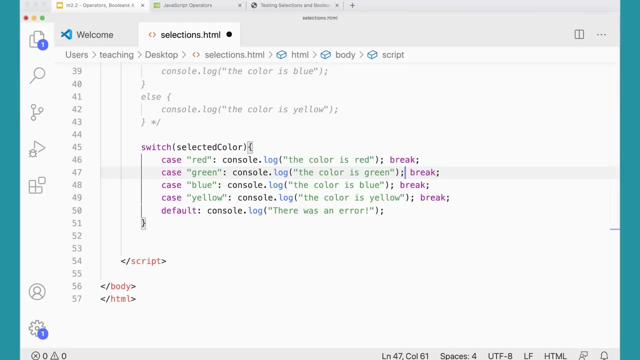 So I have to be in a good mood and have gotten sleep in order for today to be a good day. If either one of these is false, then I'm going to be gone And I'm going to be grumpy. So let's just test this one really quickly, because I think it's just a good idea to practice typing these. 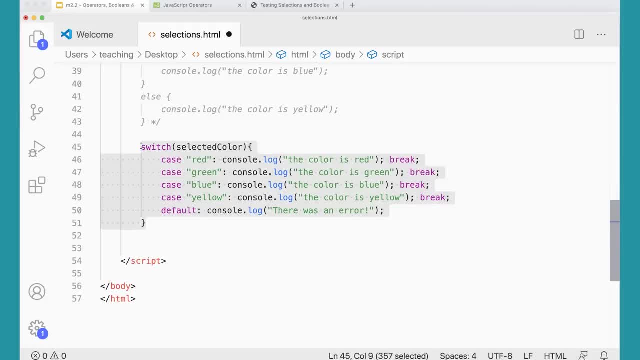 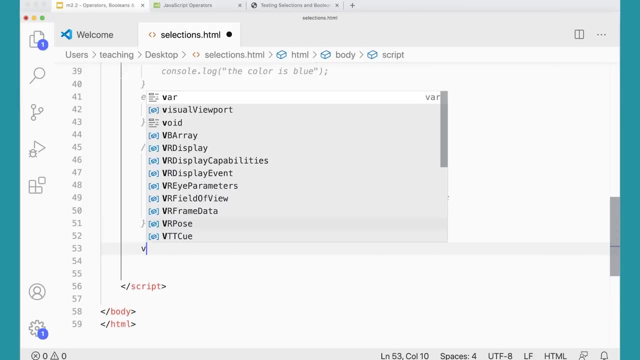 So I'm going to come in here, I'm going to turn this one off Again option or alt shift A Comments it out, And then I'm going to do var good mood And set that to true. Var got sleep. 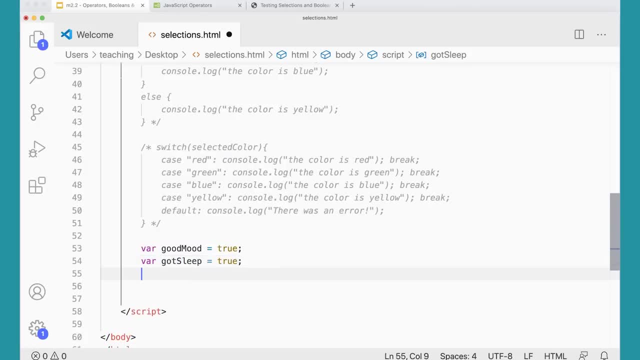 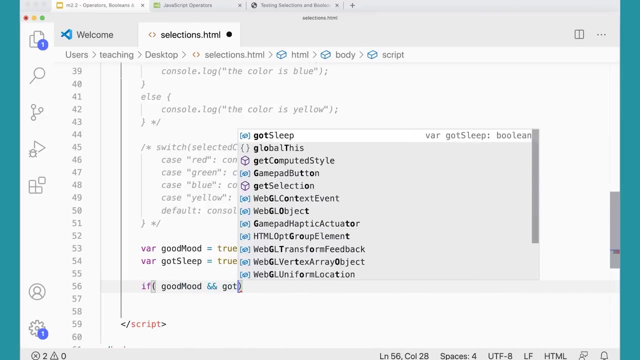 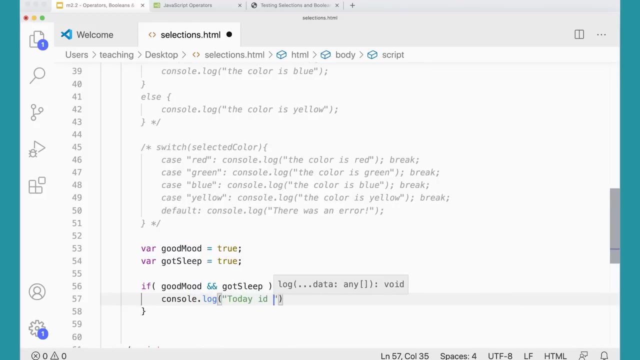 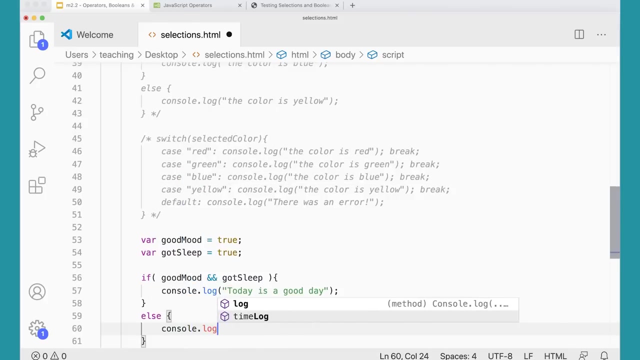 And set that to true. And then I'm going to say: if parentheses good mood, ampersand, ampersand got sleep. If both of those are true, then I can console log. Today is a good day, Else consolelog. I am grumpy. 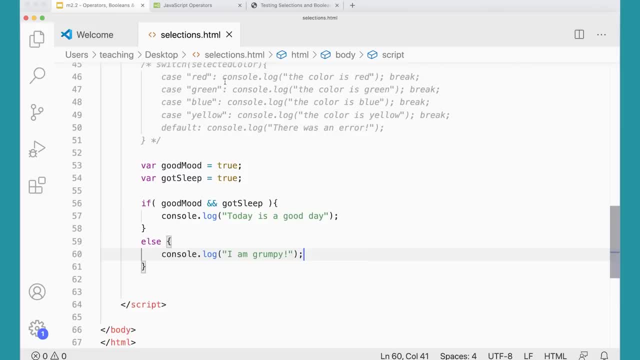 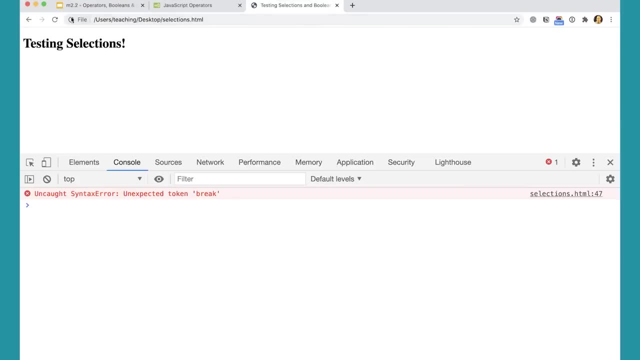 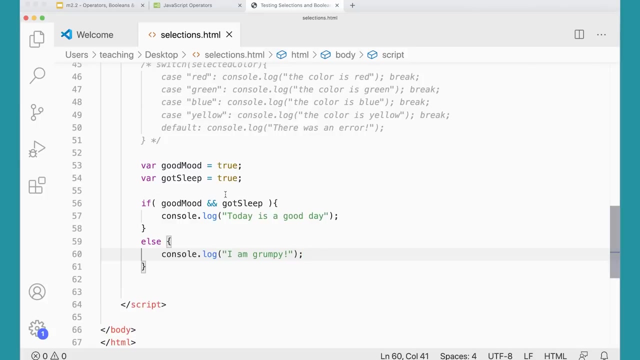 Now we can test this And we can see that, because both of these are true, because both of these are set to true, the if statement is going to run. Today is a good day, However, if I were to go in and change it so that one of these was false, 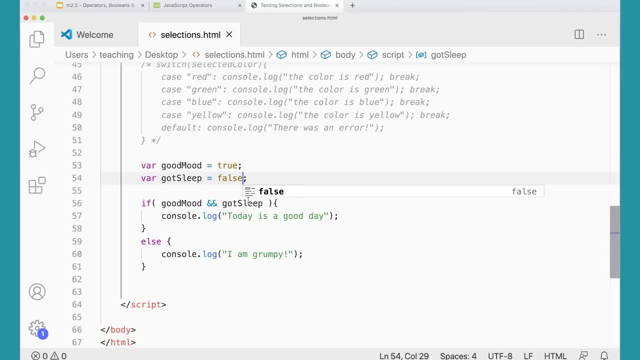 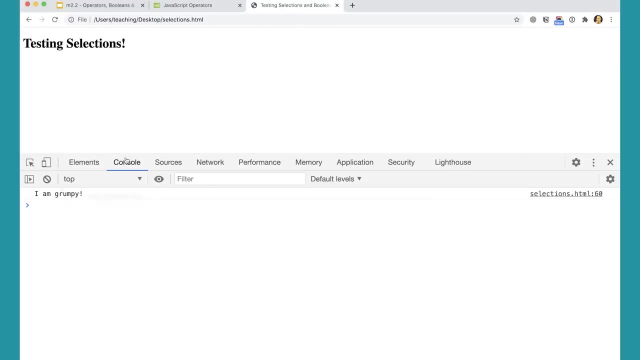 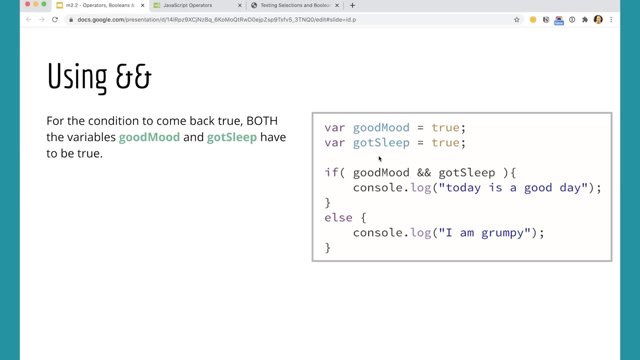 it doesn't matter which one, then this whole statement will come back false, And I am grumpy. So that's kind of an important tool in our toolkit is we can check to see if two things are true. If two things are true, then we can do something. 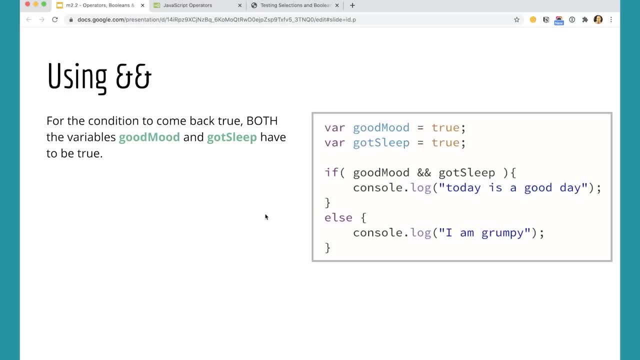 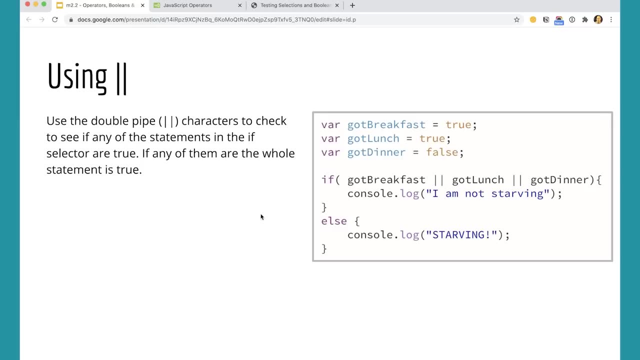 If either one of them is false, then something else is going to have to happen. Now we can also use the double pipe. The pipe is the key on the American keyboard above the return key, Shift, and that key up there It's also got the backslash on it. 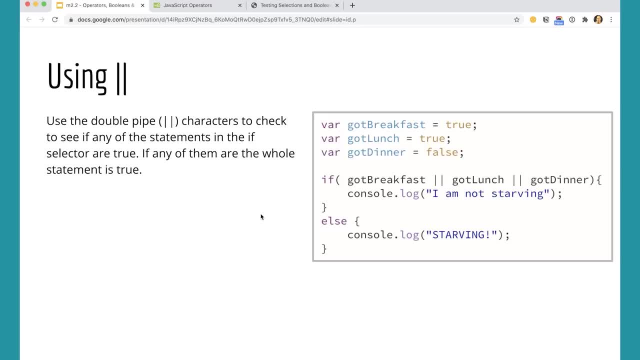 Okay, So we can also use the pipe. And the pipe is different in that it's an or statement. So here: got breakfast is true, got lunch is true, but got dinner is false. But if any one of these is true, then the if statement rings as true. 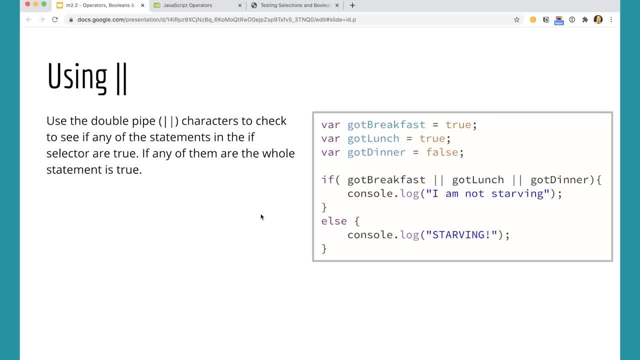 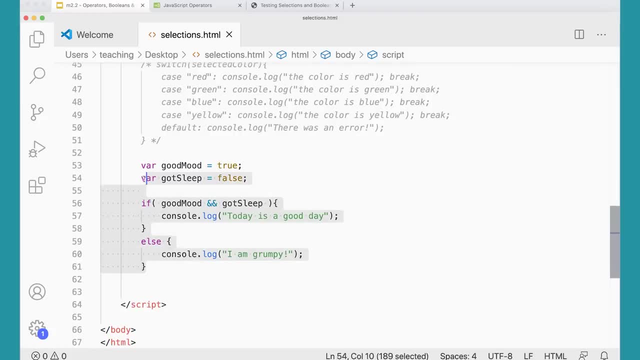 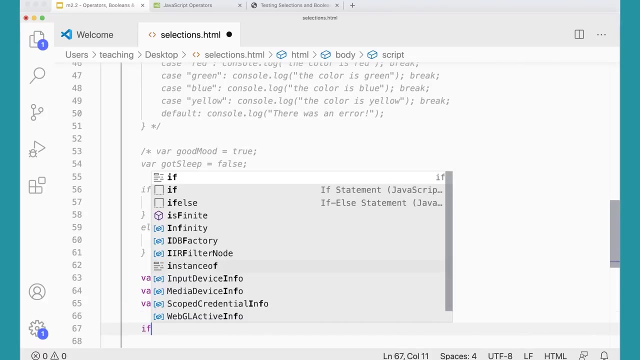 So they would all have to be false for me to be starving. Let's give it a try. Comment all this out: Bar got breakfast equals true. Bar got lunch equals true. Bar got dinner equals false. If got breakfast or got lunch or got dinner. if any of those is true, then consolelog. 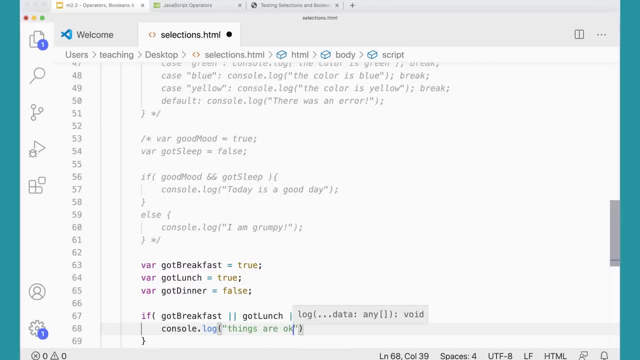 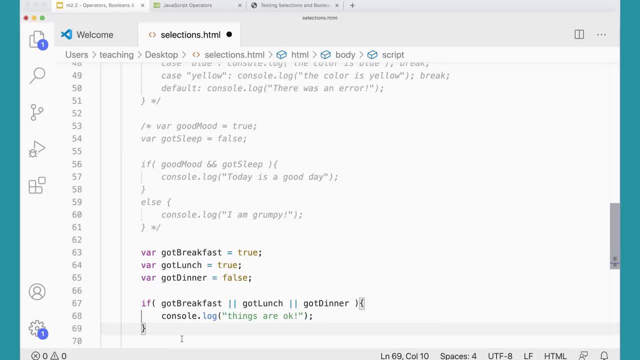 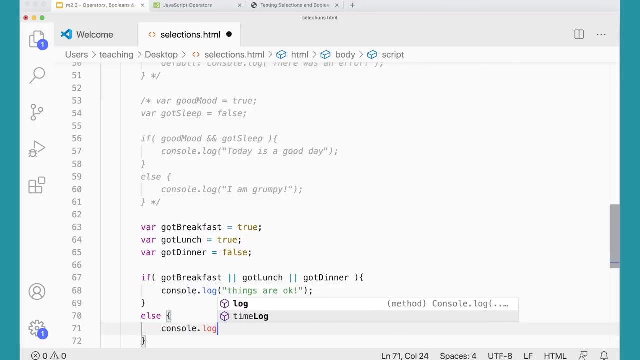 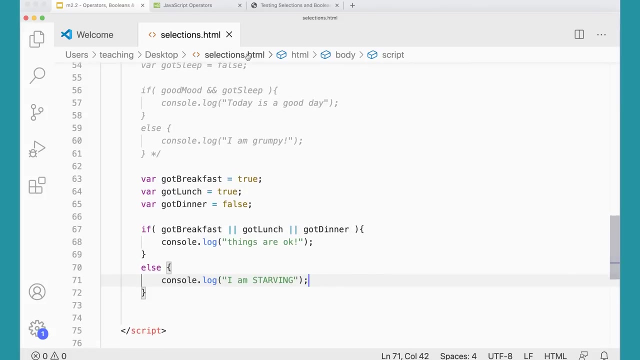 Things are okay. I forget what I put on my slide, but that's good enough. And then down here else Consolelog. I am starving And there we go, So I can test this over here And you can see things are okay. 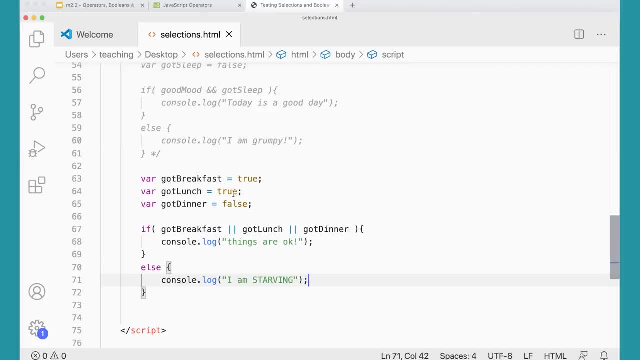 Even though one of those was false. I would have to make all of these false to really be starving. And there we go. Great, You've learned a lot about Booleans in this lesson and what's true and what's false, And that some things are true-ish and some things are false-ish, or false-y and truth-y. 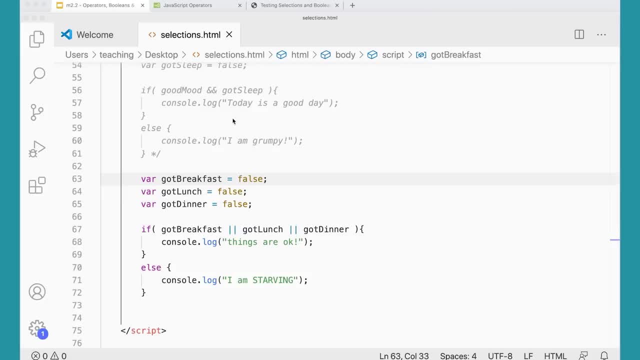 Like zero is considered false in JavaScript, or undefined, or null or not. a number is false. These are all considered false in JavaScript And you've already learned a lot of the basics of JavaScript And we're going to keep going with these basics And I know that these scripts don't seem particularly interesting yet. 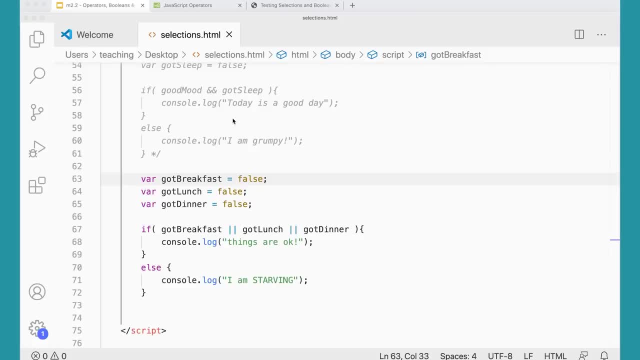 But I promise if you hang in there, you're going to learn a lot. And I promise if you hang in there and keep working on this, then we will start making some interesting things pretty quickly And we'll start manipulating content on web pages and doing all kinds of interesting stuff. 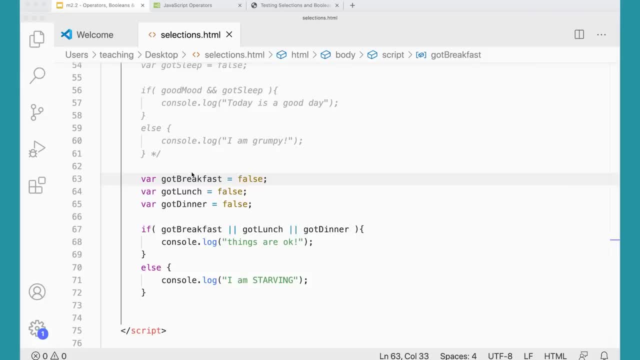 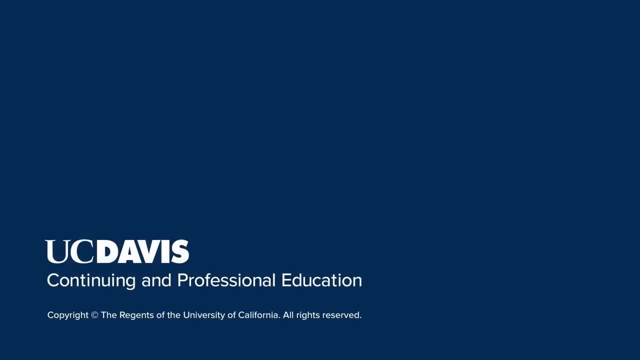 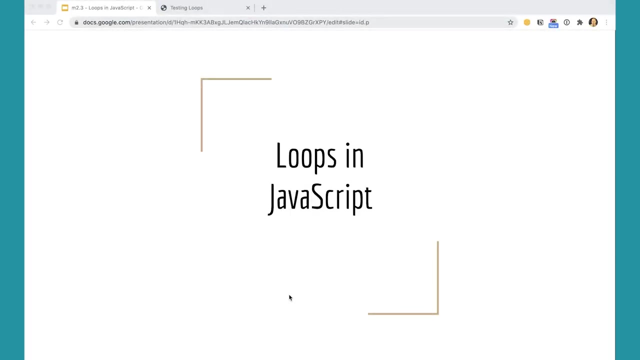 So hang in there, Keep going, And if you haven't had breakfast, lunch or dinner, you're probably starving, so you should go eat. something Loops in JavaScript. We've already done quite a bit of JavaScript already. We've looked at variables and we've looked at arrays. 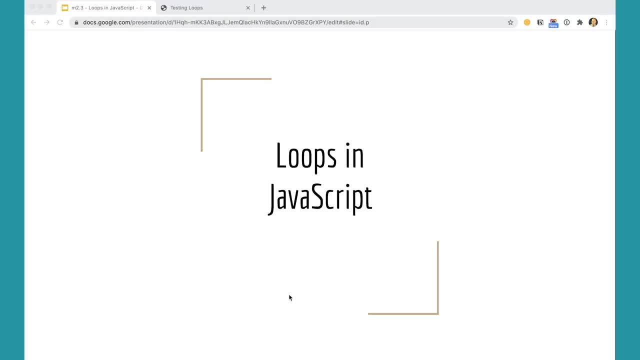 And we've looked at how to use selections to choose if something is true or not- Booleans. The next piece of the puzzle is loops. Frequently, you need to iterate through a number of values and do something with them when you're programming, And JavaScript, like many programming languages, will allow you to do loops. 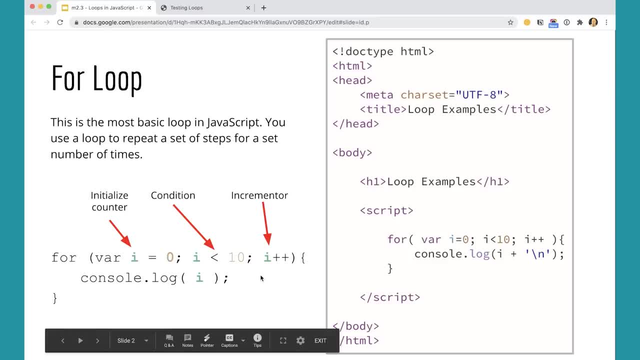 The most basic loop is a for loop, And you'll see here that in the for loop we start out with an initialized value And then we check if the value is less than some number And then each time through the loop we increment that value. 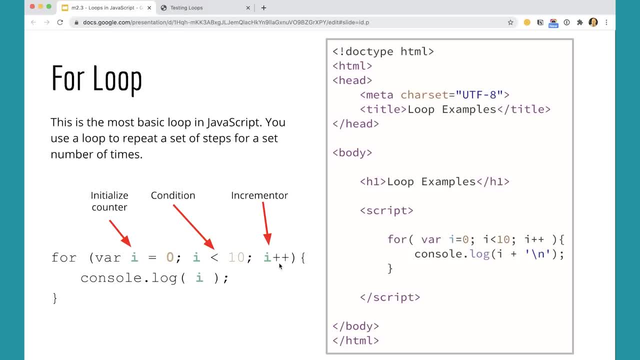 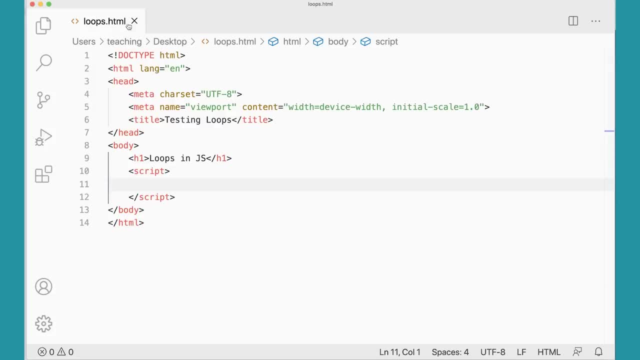 The best way to explore this is to actually try it out, So I recommend opening up your code editor and following along with me Here. I have just a file called loops. I'll save it on my desktop And I'm going to add a loop in this script down here. 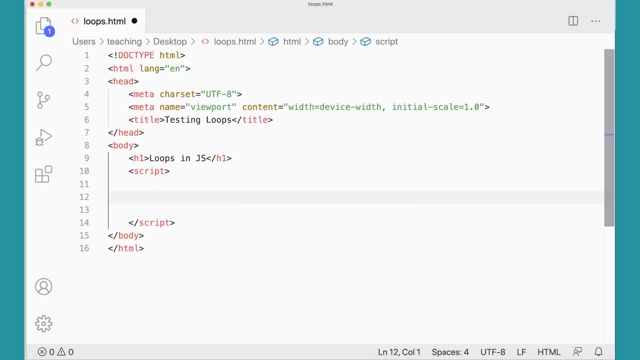 So over here I'm just going to make a little room here. There we go And I'm going to add a for loop And there we go, And then in here I'm going to just make a little space there so it's a little easier to see. 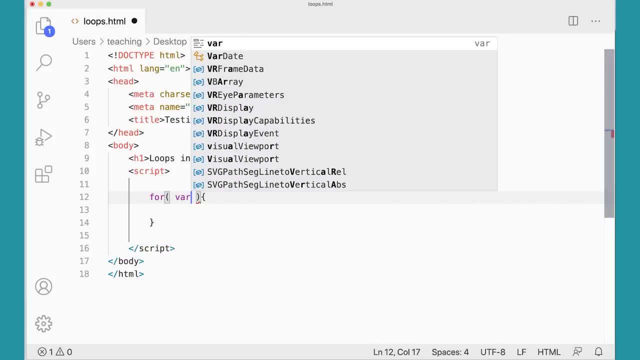 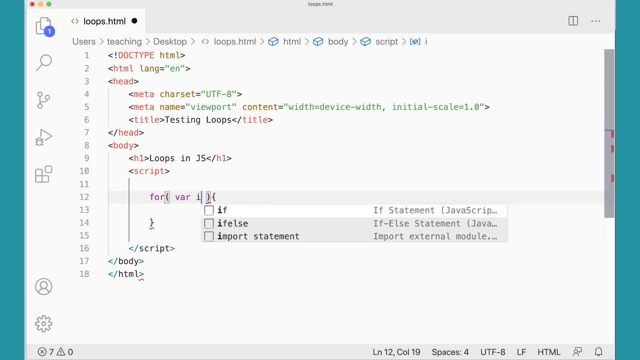 But I'm going to make a variable, var i And i can be anything. It could be x, It could be y, It could be j, It could be the word counter. It's just a variable i is fairly common to use because it can stand for incrementer. 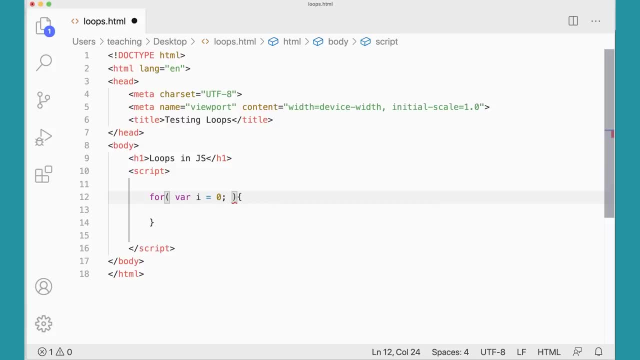 I don't know, It's a fairly common one to use, But it doesn't have to be that. It could be something else if you want. But I'm going to start i at 0. And then I'm going to check while i is less than, say, 10.. 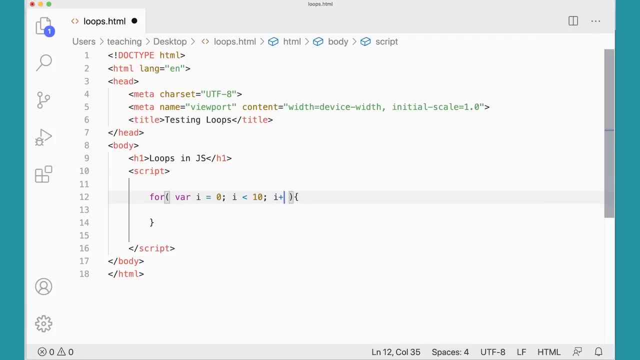 And then each time through the loop I'm going to increment i, i++. i++ is a shortcut for i equals i plus 1, like so. So we could take i add 1 to it and then assign it back to i. 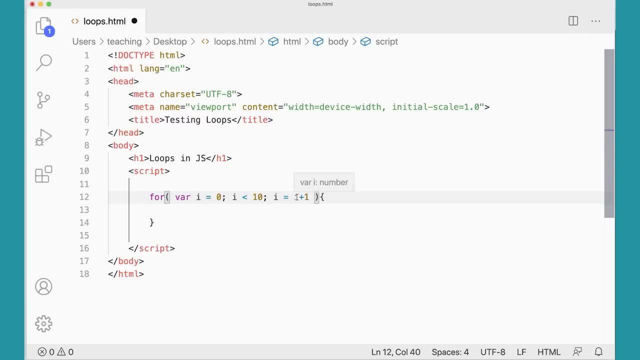 So if i starts at 0,, the next time through the loop we'll take 0,, add 1 to it, which gives us 1, and assign it back to i. So now i is 1.. And then the next time through the loop we'll take 1,, add 1 to it, assign it back to i. 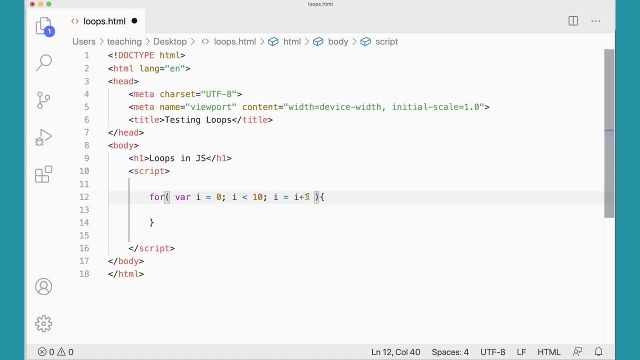 So now it's 2.. So on and so forth. But a shortcut for that is i++. So that's an incrementer, OK, great. So there we have it. And then here we have, let's just do consolelog i, not 1, i. 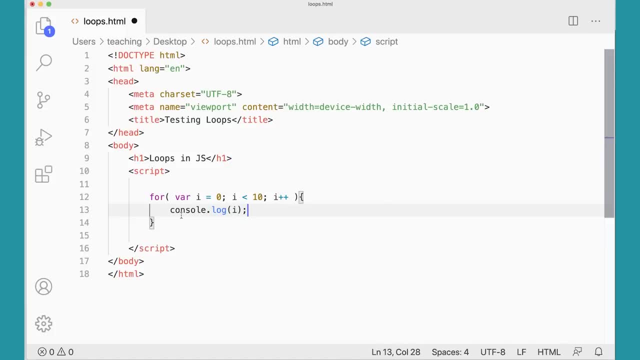 There we go, And so what this is going to do is we're going to set i to 0.. 0. So the consolelog will run And it will say it'll give us a 0. And then we come back and we increment i so that we take 0 and we add 1 to it. 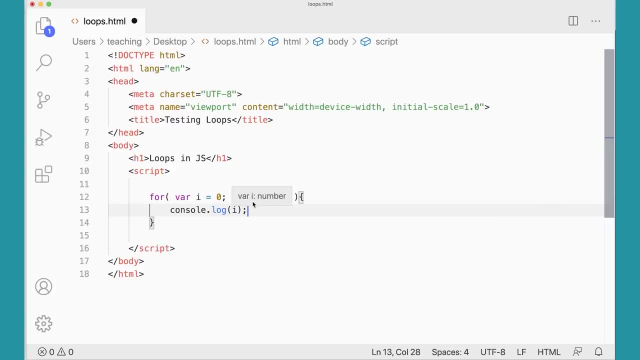 So now it's 1.. Is 1 less than 10? Yes, it is. Since 1 is less than 10, it will consolelog i again, which is now 1. And then it'll increment 1 again. 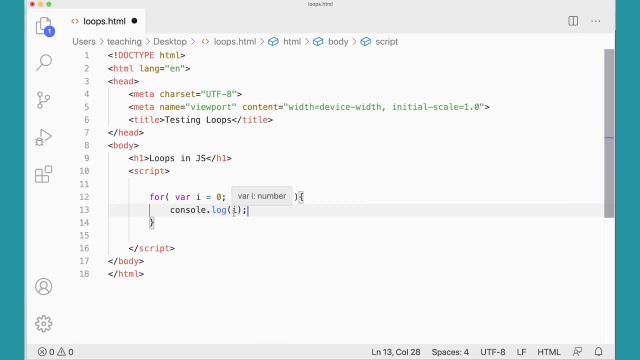 So 1 will go from, i will go from 1 to 2.. And then is 2 less than 10?? Yes, it is. So we'll consolelog out a 2.. And then we'll increment. i again, We'll take 2 and we'll increment it to 3.. 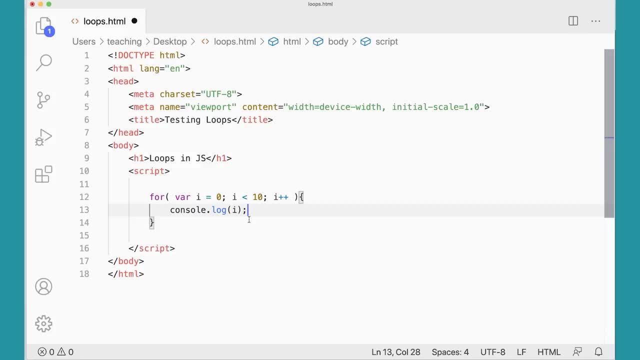 Is 3 less than 10?? Yes, it is. We'll consolelog out a 3.. And so on and so forth until we get to 9.. When we get to 9,, we'll consolelog out the 9.. 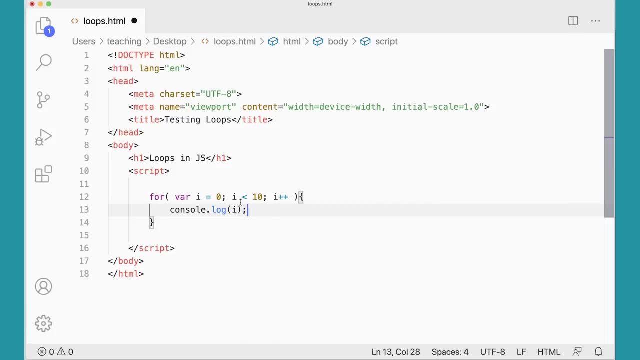 And then i gets incremented to 10.. Is 10 less than 10?? No, it's not. So then the loop will stop and will bust out of the loop at that point. But let's give this a try. I'm going to save this. 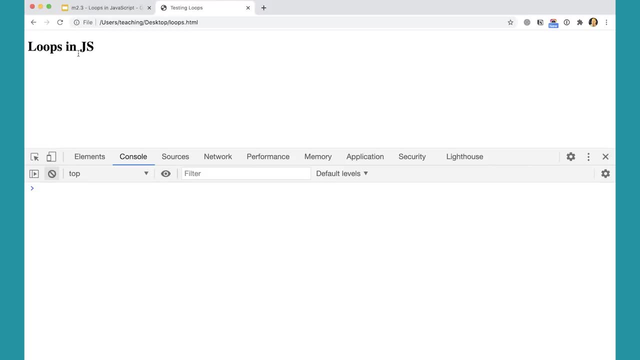 And then I'm going to go to the browser which I have over here And I have this file loaded here And I can just run it And you'll see that my loop ran. Line 13 ran 10 times, starting with 0.. 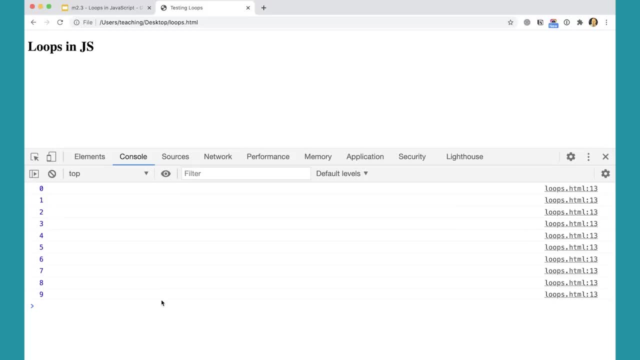 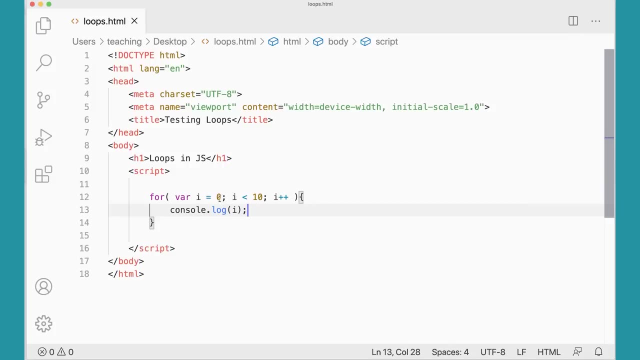 0 through 9.. So that works and that's great. Now I don't have to start with 0.. If I wanted to count from 1 to 10, I could start with 1 and say, well, i is less than 11.. 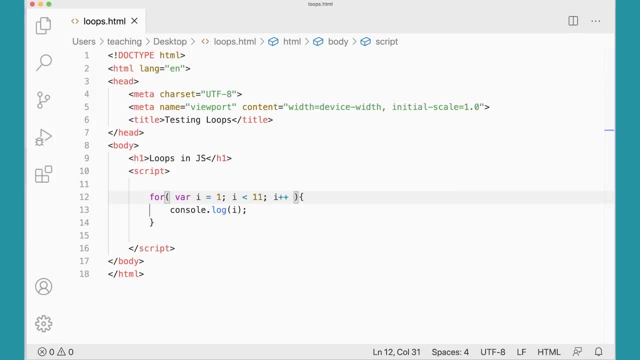 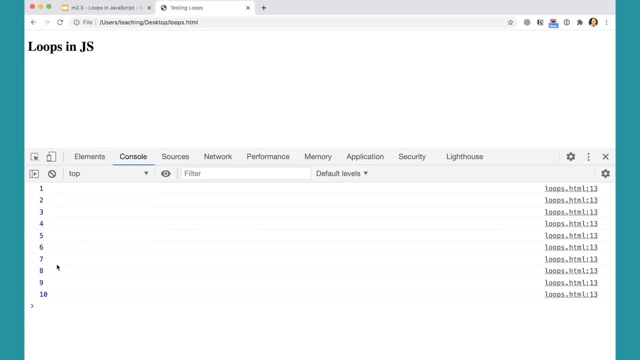 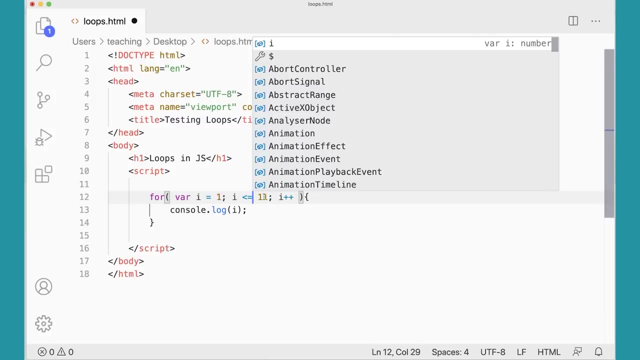 And that'll work just fine. And now I've got a 1 to 10. I could even say: well, I want it to be less than 11.. I want it to be less than or equal to 10.. So then that'll actually work as well. 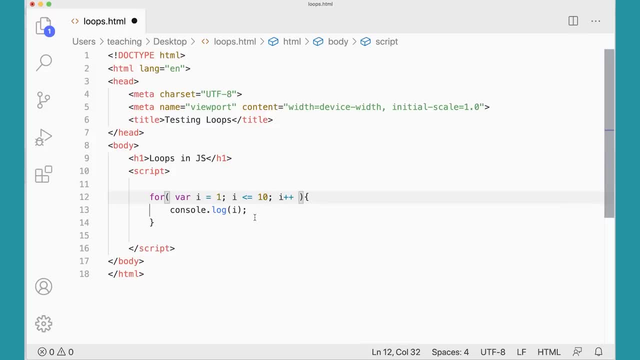 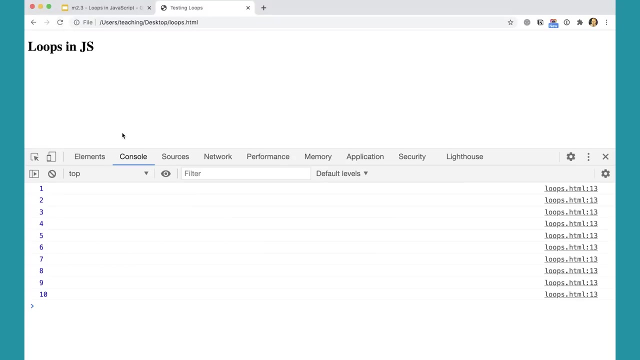 So that's less than or equal. That's a less than or equal operator. Greater than or equal would be this one. But we want less than or equal And you'll see I get the exact same result. You also don't have to start i at 1 or 0.. 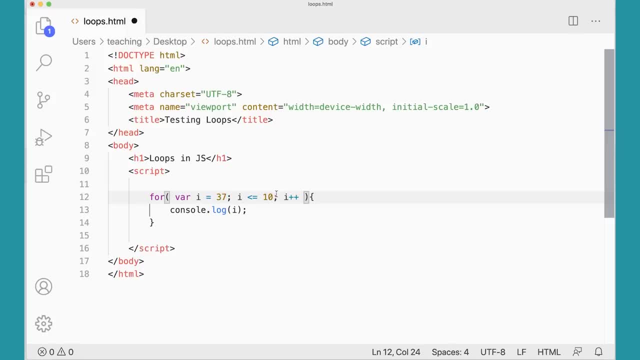 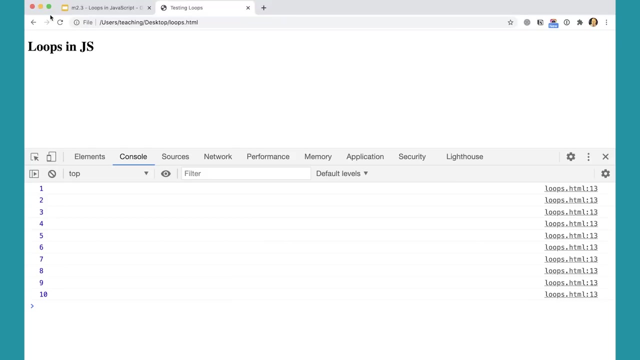 You could start i anywhere If I wanted to. I could start at 37 and go till I'm at 63, if I want to. i plus, plus, And then if I go back and do that, you'll see that the loop will do those numbers. 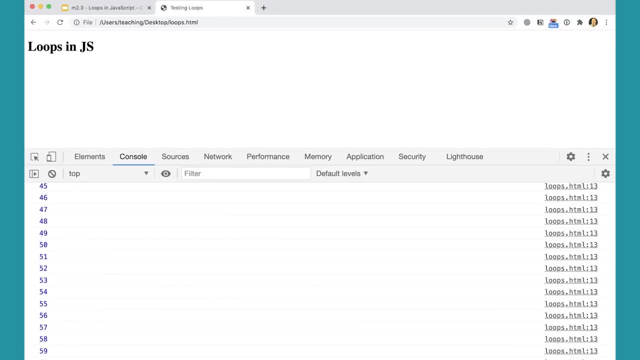 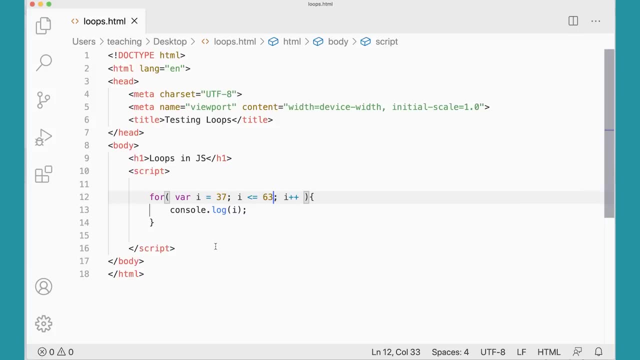 So there are a lot of different ways of creating loops in JavaScript And we'll be looking at a few different methods throughout this course, But the for loop with these three expressions is really your most basic loop And as we go through the loop, we evaluate these expressions. 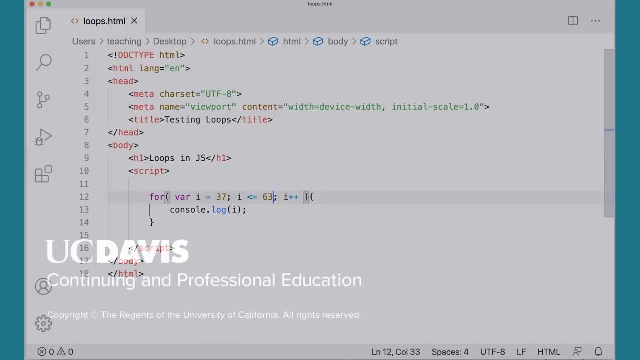 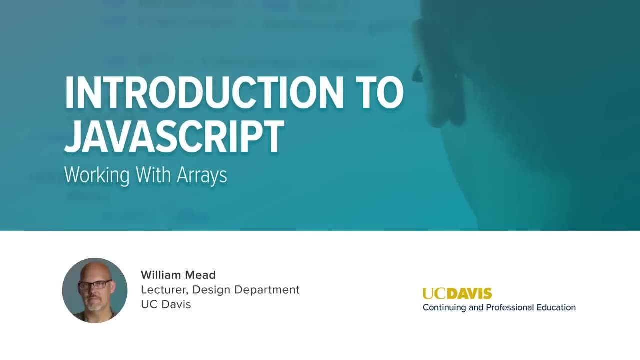 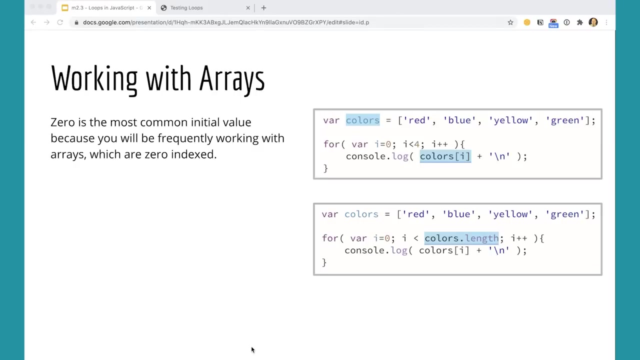 And that determines whether the loop runs or not. One of the places you're very likely to come across using loops is if you have an array of items. You have a group of items and you need to iterate over that group of items to do something to them. 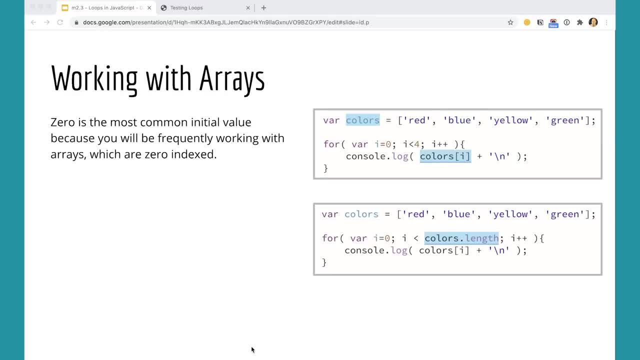 And so let's take a look at what that looks like. Here I have a variable called colors, which is an array. It's got red, blue, yellow and green in it, And then I'm going to loop through Each of the colors in the array. 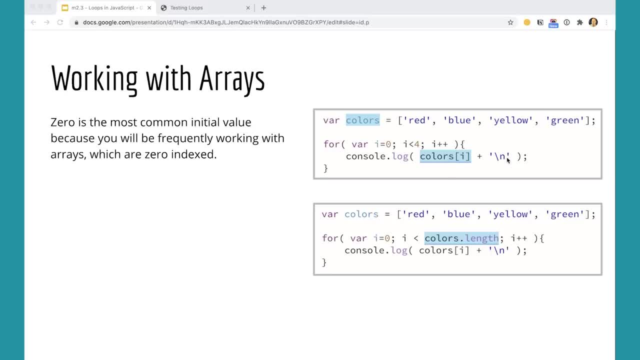 If you're wondering what this plus quote slash n is, that's to create a new line in the console, And actually I don't really need to do that because in fact the console creates a new line for each call anyway, So I shouldn't have put this on my slide here. 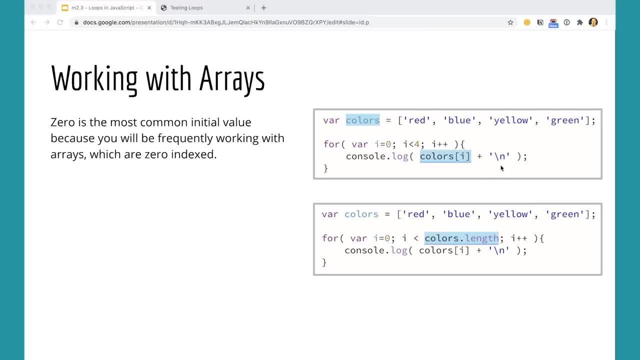 But I forgot to take it off. But you can just ignore it. We can just do it without that And it'll work just fine. So remember a razor zero index. So this is a zero index. This is element zero. This is element one. 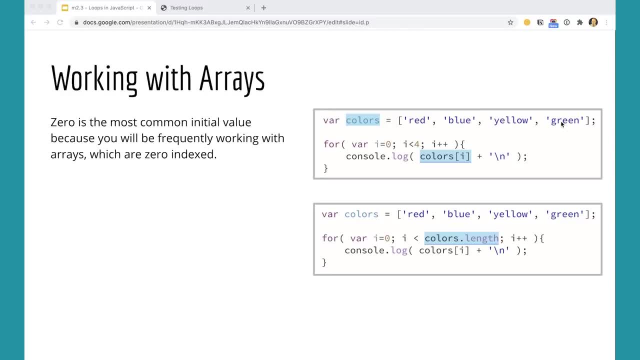 This is element two. This is element three. The length of the array is four, But zero, one, two and three. So let's go over and give this a try really quickly. Here I am on the same file I had before. 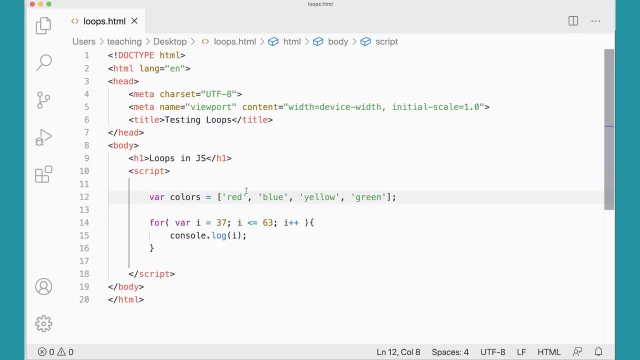 I didn't update my loop, but I added the array with the colors in here. So what we would do down here is we would set i to zero first, So we'd get red, And then, while i is less than four, while i is less than four, 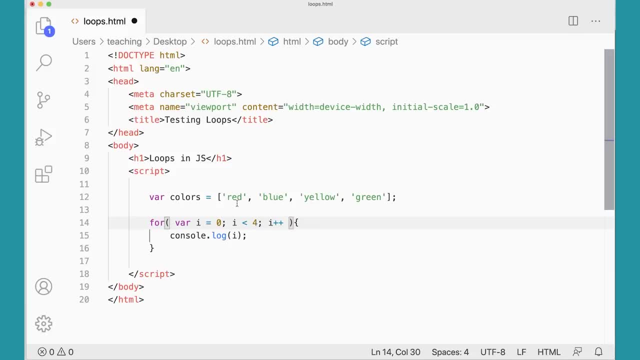 And then we're going to increment i because we're going to do it for red, blue, yellow and green. And then down here I'm just going to console log out colors: square bracket i. So the first time through the loop i is a zero. 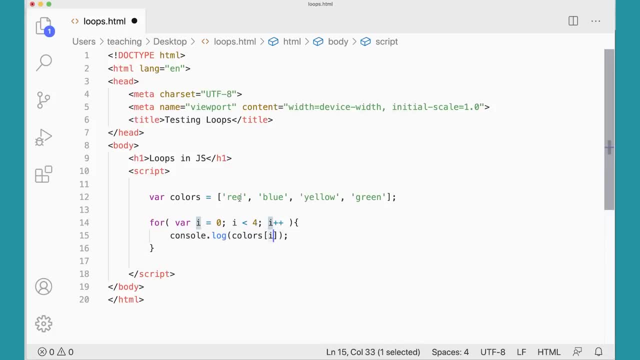 Colors- square, bracket zero gives me a red, And then i gets incremented to one. And the second time through the loop i is a one. I go to my colors array here. Colors- square, bracket one gives me a blue, i gets incremented to two. 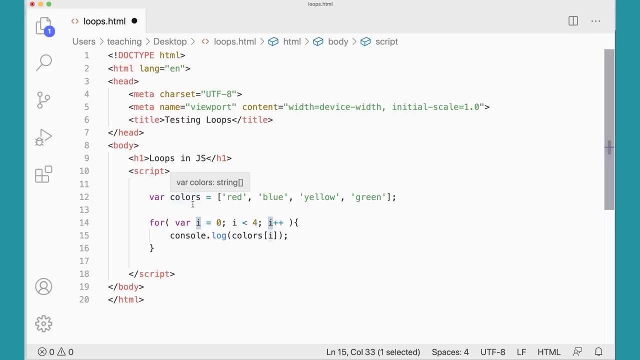 So I go up to colors here and I go zero, one, two. Now colors: square bracket two is going to give me yellow. i gets incremented to three Colors. three is zero one, two, three. It's going to be a green. 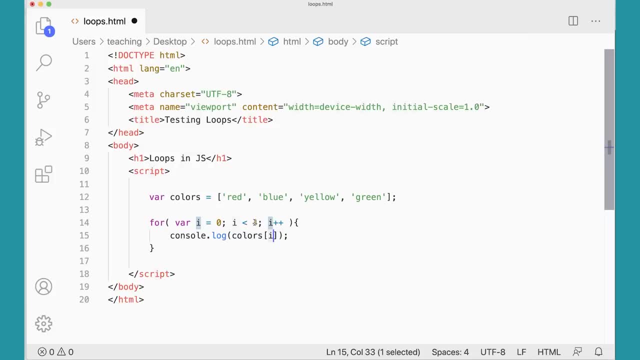 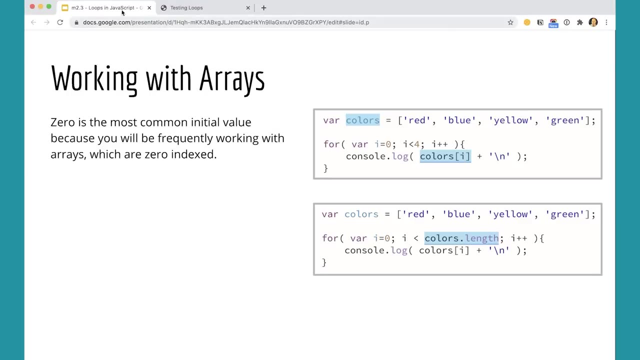 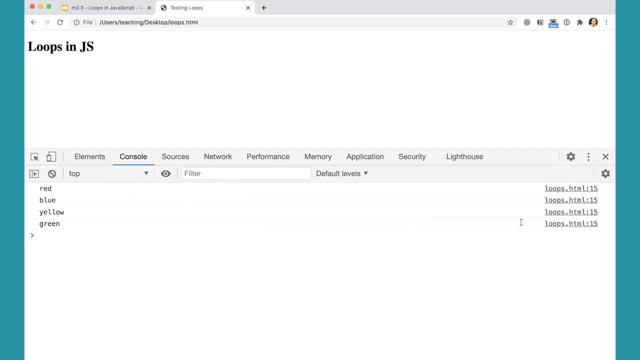 i gets incremented to four- Four is no longer less than four- And my loop breaks out. Let's give this a try and see if it works. And sure enough, I get my four colors out in the array And it's looping through and doing line 15 four times. 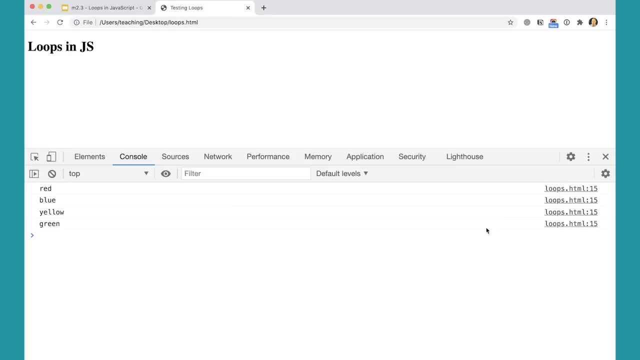 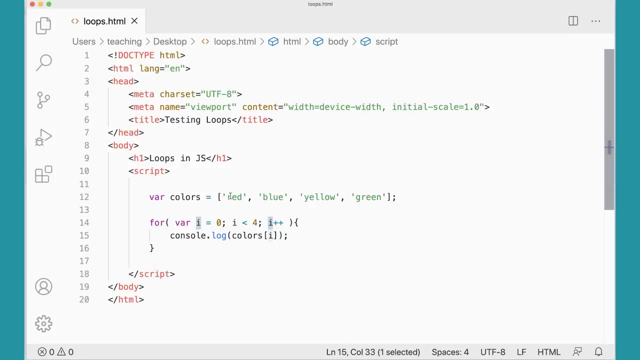 Four times there, So that's really useful. Now, generally this is fine, This works, But generally we don't want to have to put in a number here. What's better is to keep this more general. So if I do colors dot length, that's also a four. 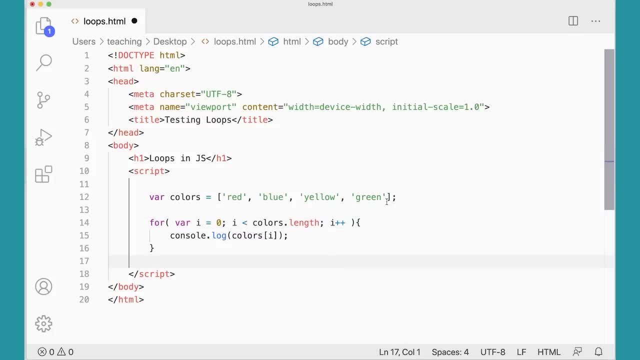 Colors: dot length is a four. I could add more colors into my array and this code will still run, No matter how many colors I have in my array. I could add in here orange and purple into the array And this will continue to work, because now the length of my array is six. 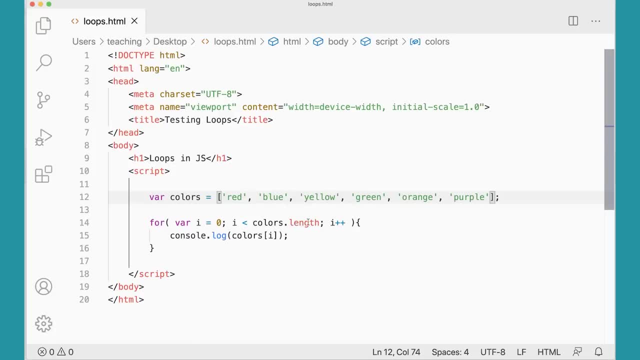 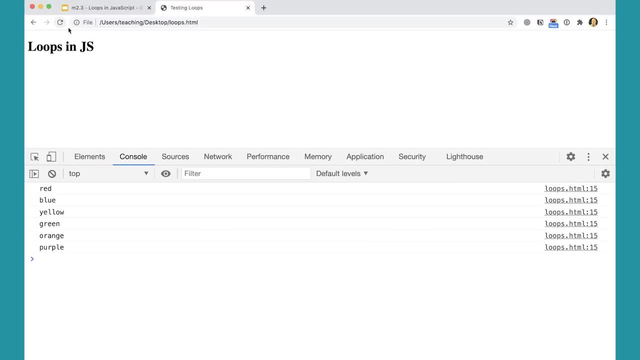 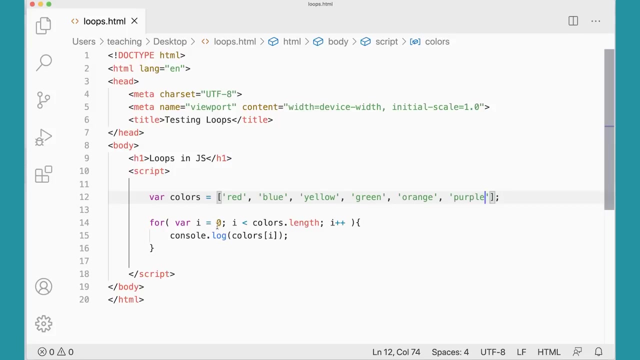 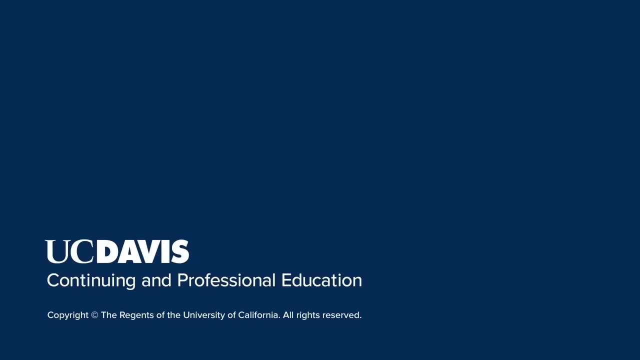 So I don't have to update this number every time. Colors dot length will help me make my code more general And allow me to do that kind of thing more easily. Okay, So we can do that really nicely And loop through all the colors in the array that way. 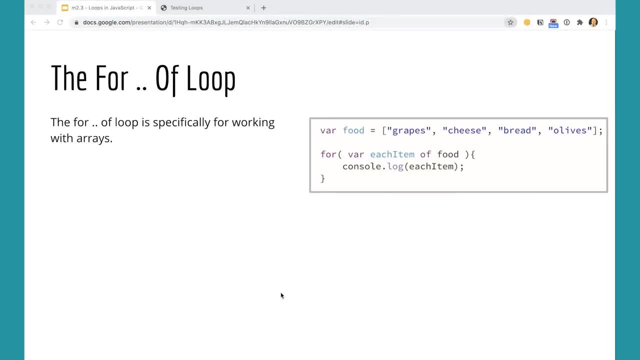 The basic for loop is a good place to start With loops, But there's also a loop that is specifically for working with arrays And it's called the four of loop, And here I have an array of food And you can see there are four items in here. 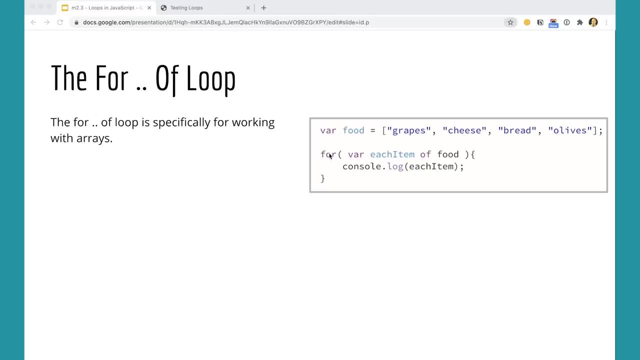 Four foods And I can use four, and I can create a variable, A temporary variable, And I'm calling it each item. But you could call it x, You could call it y, You could call it whatever you want. Each item of food. 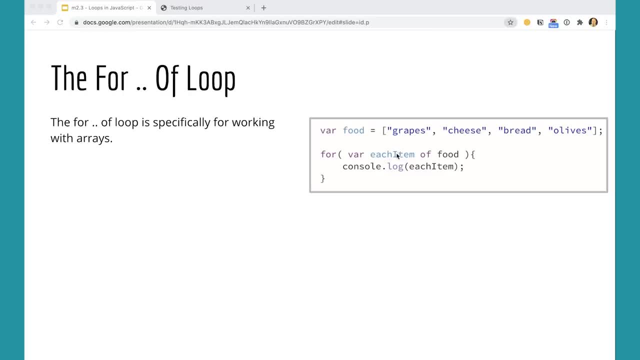 So each item. what this loop is going to do is it's going to go through this array until the end of the array And each item the first time through the loop is going to be grapes. So I'll consolelog out grapes And then, since the array has not reached the end yet, it will run again. 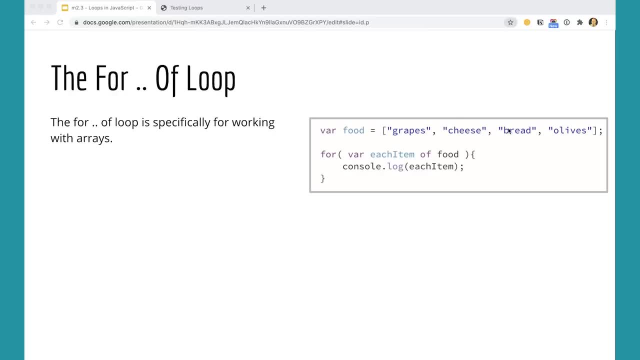 And each item will become cheese, And then it will become bread, And then it will become olives. So let's give this a try really quickly Over here, in our code over here, And I'm going to just leave the array with colors. 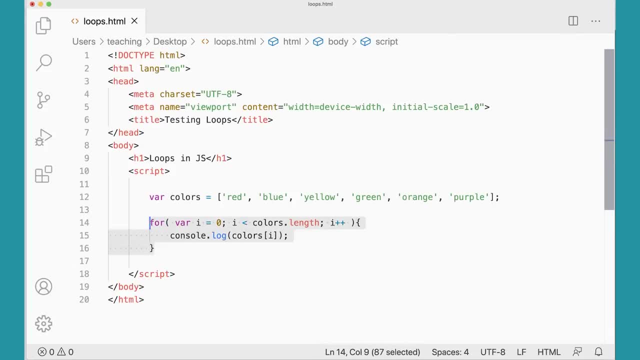 But instead of this for loop, I'm going to do for var, each color of colors And it knows what colors is because that's been defined here: Each color. I'm putting var here because I'm creating a variable, Because I'm creating a new variable there. 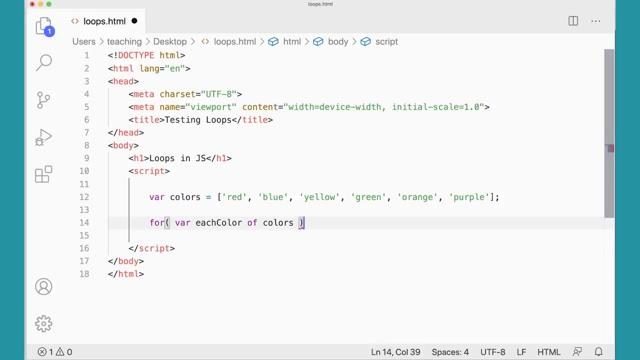 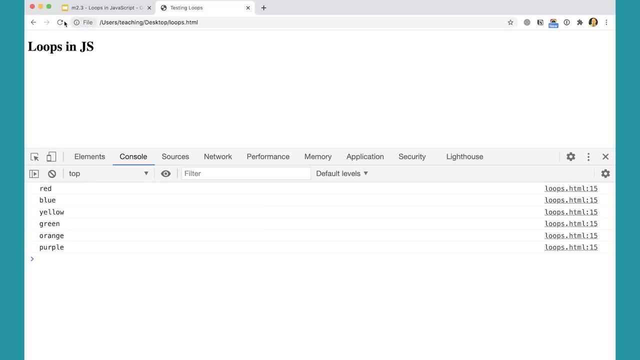 And then down here I can- actually I wanted to put the curly brace there. Down here I can do consolelog. each color, Oops. And you'll see that when this runs over here I get each color, I get the same thing. 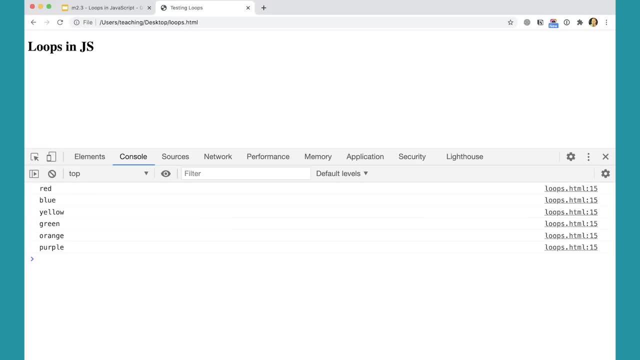 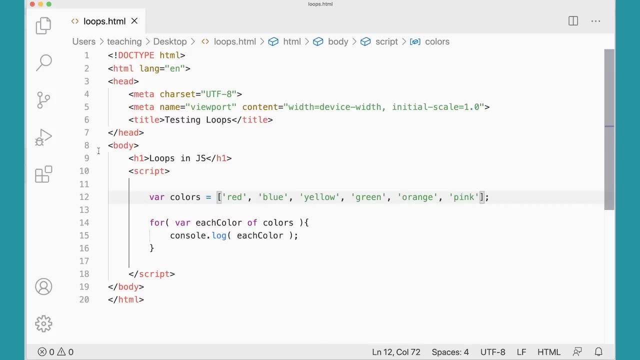 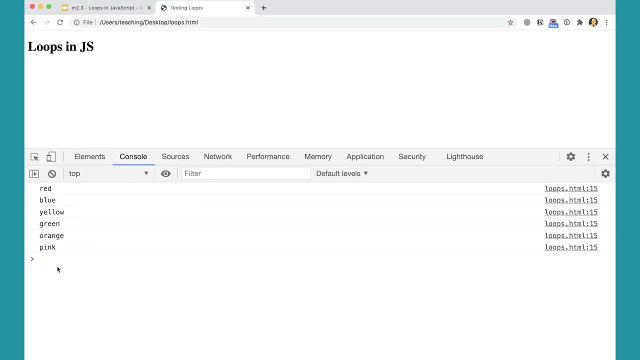 It doesn't look any different. It might be kind of nice to actually make it. do something a little bit different And come over here and change purple to pink, Just so that we can see that it is actually doing something. Refresh this, And sure I get them all again with pink instead. 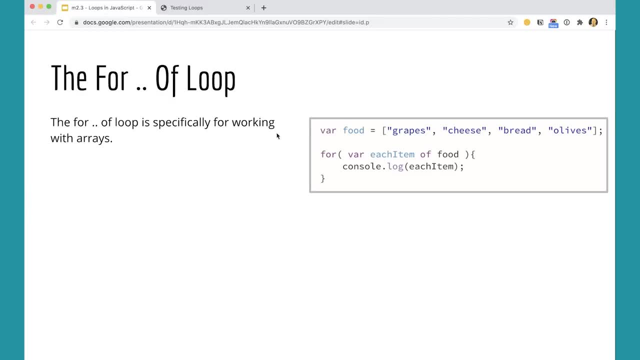 Okay, So that is actually working. This is a great tool to use with arrays. There's another one called for in that we'll talk about later, With objects, But for of is specifically for arrays, And then there's another method that we'll be looking at that also works well with arrays. 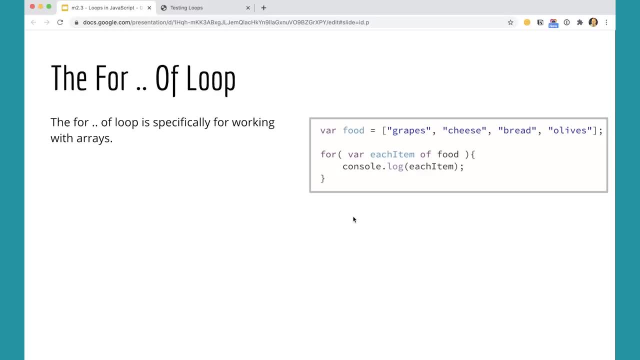 That I use a lot when I'm programming JavaScript. I tend to use the for each method, But we'll look at that later in the course. But right now I just want to get you started with the basics So you can see how to do this. 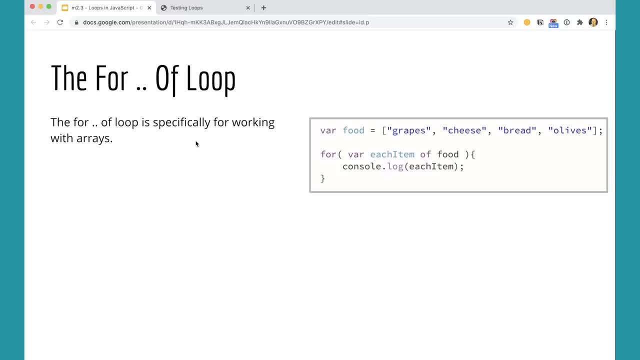 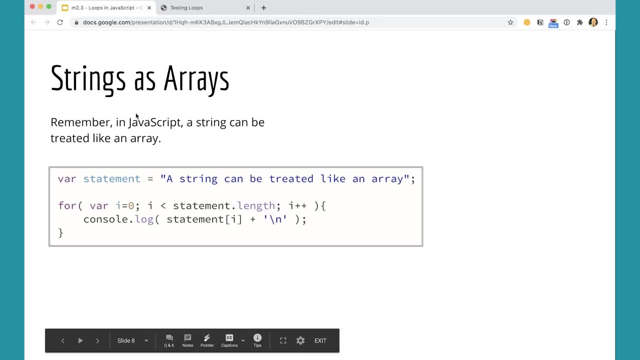 And the basic for loop is a good place to start For of is great for working with arrays. There's also we can also do something with strings, So we could actually remember strings are treated, can be treated like an array, So I can actually make a string and then loop through the length of this thing. 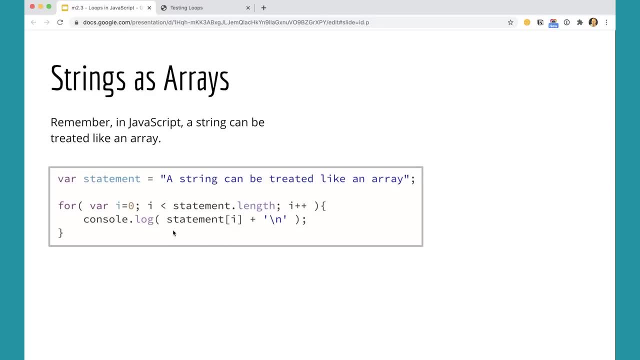 And actually alert out. You know each letter one at a time in my, in my console log there, So I can do that kind of thing. In fact, let's give this a try really quickly here. I'm going to change this to. 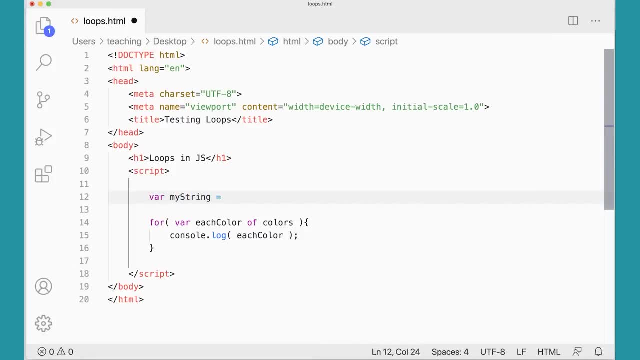 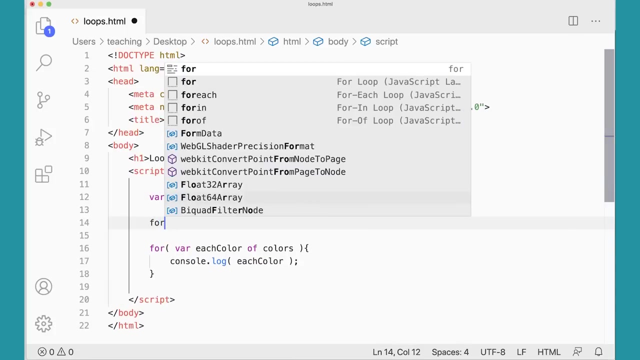 My string Equals. Here Is a is a string of Text. There we go, And I could do it. I can do it this way, for For I Equals Zero. Well, I is less than My string. 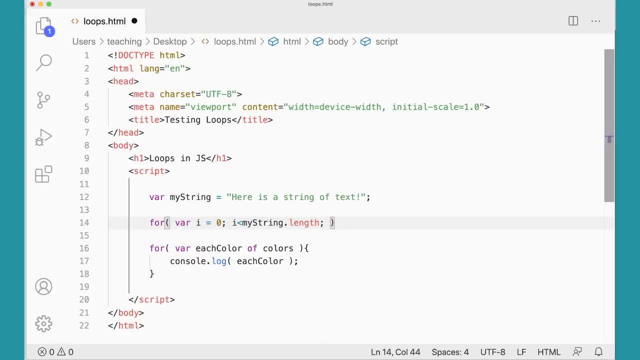 Length I Plus Plus Console Log My String Square Bracket I, So I can do it this way. Comment this out. for now That should work. If I didn't type it wrong, Let's see if I did it right. 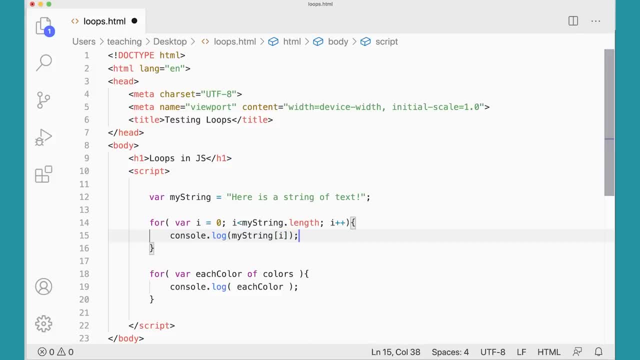 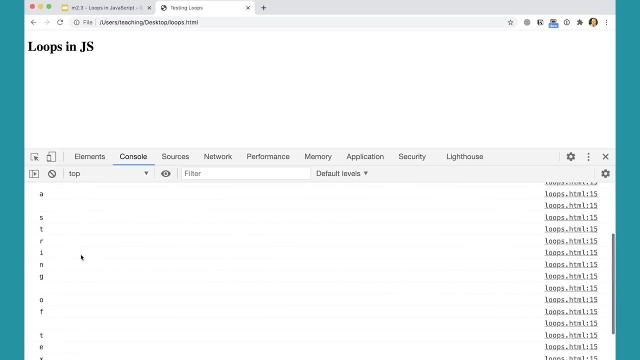 So I Plus Plus Console Log My String Square Bracket I, So I can do it this way: Comment this out for now, And sure enough There's. Each line has a letter, So I could do it that way. 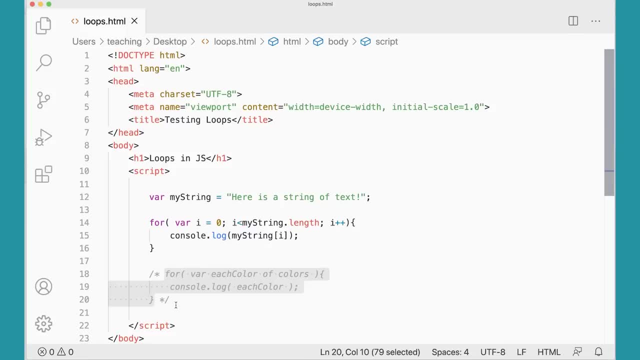 Or I could even use the for of loop. So I'm going to, So I didn't delete this, So I can actually Take this Uncomment, this out, And instead of Each color, I could do Each Letter Of. 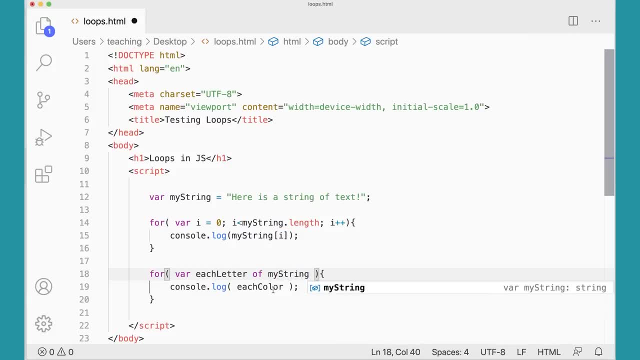 My string Each Letter. That'll work too. Now I'm going to get it twice. I'm going to get The loop twice. I'm going to get the first loop, which is the first one, And then I get the second. 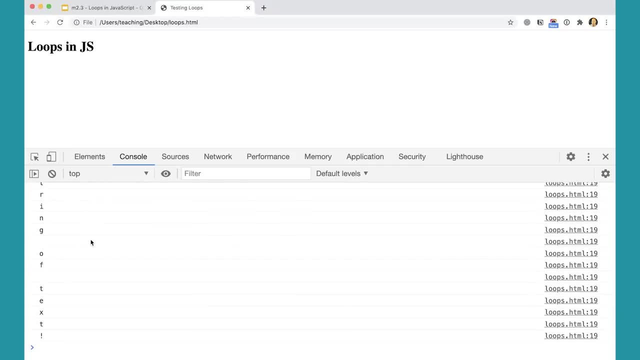 So then it's actually running twice And that's actually working really nicely. So You can actually treat a string Like an array In that way. I'll do this. I can If I Really like My string Okay. 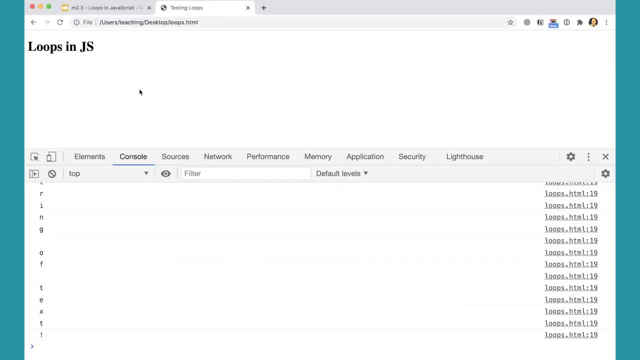 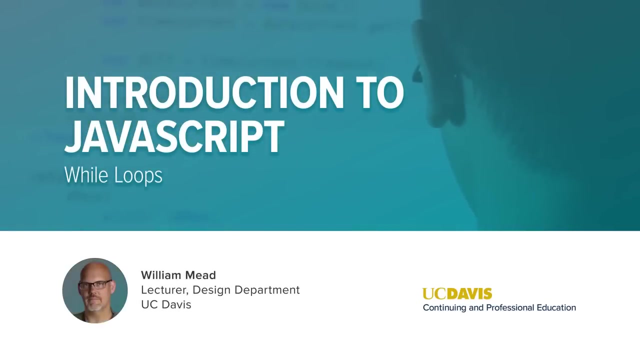 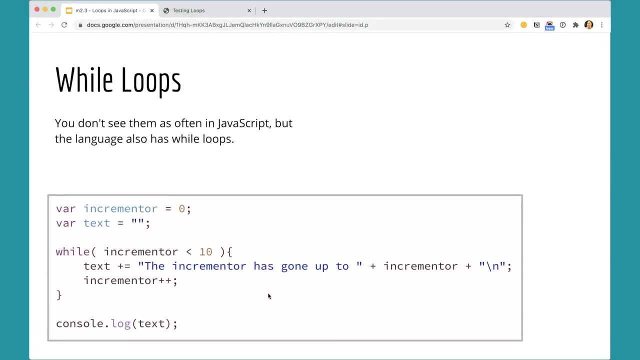 So I Can Use This in that way and that's. that's really kind of a very interesting feature of javascript. javascript also has a while loop, and we don't see them as often while we're programming with javascript, but they're worth knowing about, so let's take a look at them really quickly. 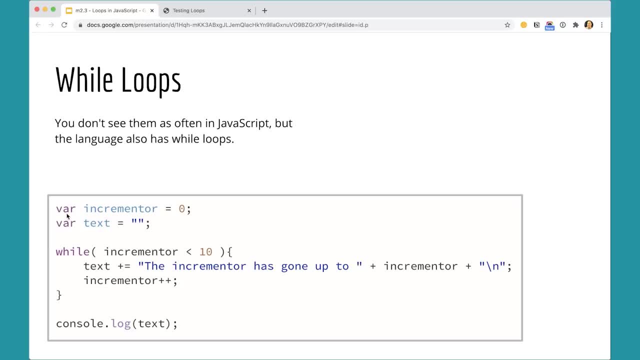 and here we can see the way the while loop works is: we start off, we have an incrementer and then i'm making a variable that starts as an empty string. that's maybe not quite as necessary, but you have to have the incrementer outside of the while loop. 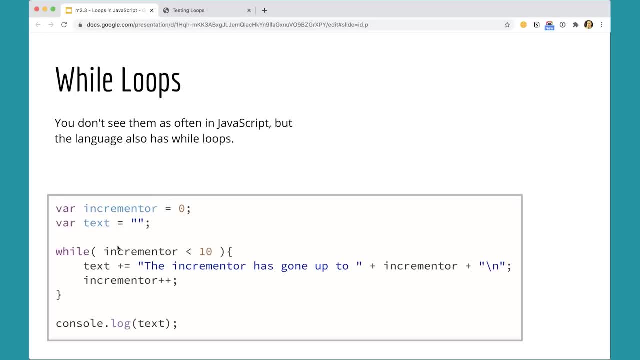 in when you're using a while loop, and then, while the while loop is less than 10, i'm going to do this stuff and then increment the incrementer at the bottom of the while loop. so this is going to run. incrementer gets set to one. one is less than 10, so this runs again. 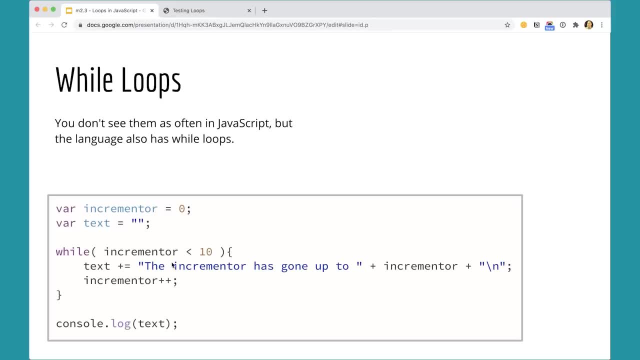 incrementer gets set to two. two is less than 10, so this runs again. so on and so forth, and then notice when the loop is done. once this increments up to 10, 10 is no longer less than 10, so i'll bump out of the while loop this console log is going to run text. what i'd like you to notice? 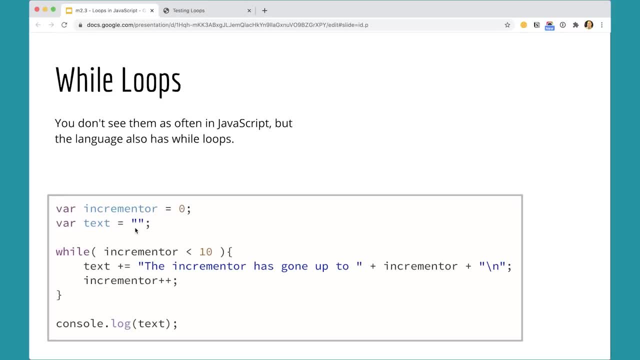 here is this: plus equals. this text is starting out as empty and plus equals is saying: each time this thing runs, add to what was there before the first time through the loop. there's nothing in there, so it's going to add: the incrementer has gone up to plus incrementer, so that's going to be a zero and then a new line. 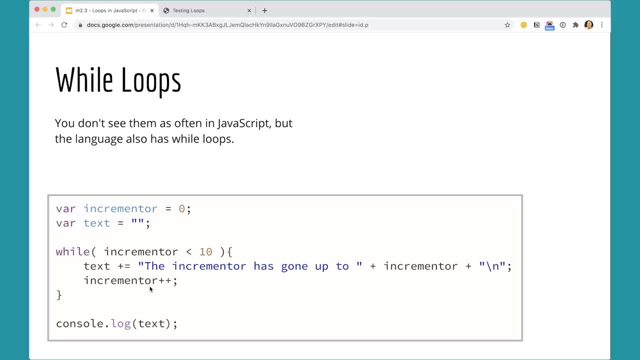 and then the incrementer gets incremented to one and then the next time through the loop we're going to add to that. so it's going to add a new line that says the incrementer has gone up to one and then it's getting increment again. then we'll say: 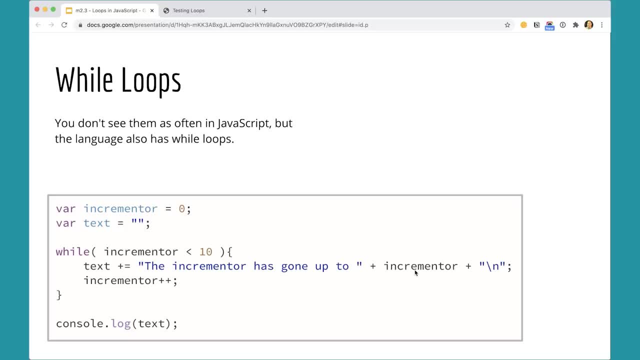 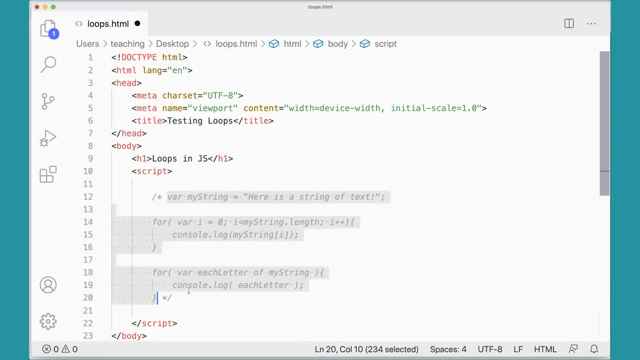 the incrementer has gone up to two, so on and so forth. let's do this one in the in the code editor, because i think it's really worth seeing this. so i've got my floor loops there. i'm just going to comment that stuff out. i don't really need that. now, come down here. i'm going to make a variable. 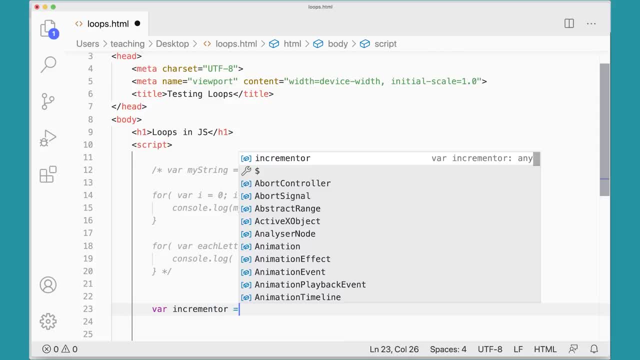 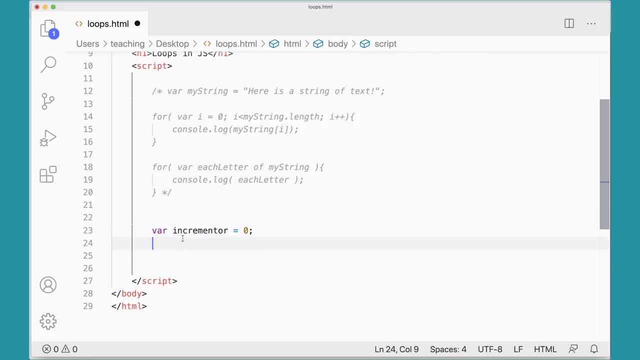 bar incrementor equals zero and again, it doesn't have to be increment or you could leave it. i, if you wanted to, that would be fine. um, and then i'm going to make var text equal quote. quote. that's an empty string. and notice, i'm using just the single quotes here, but you could do the double quotes if you. 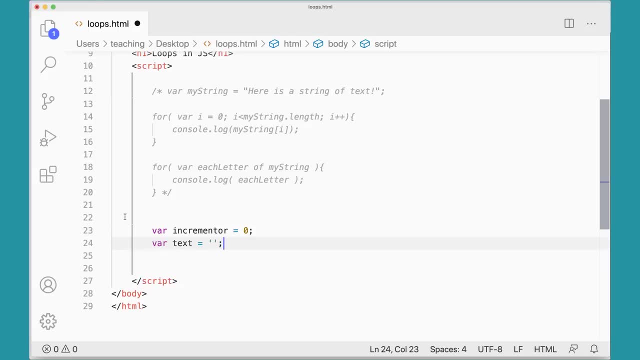 want, and the double quotes and the other, the other. um, on my image there. but you could do single quotes, i'll put it in double quotes, why not? there we go. so it's just an empty string there, and then, while incrementer is less than 10, i'm going to do something. 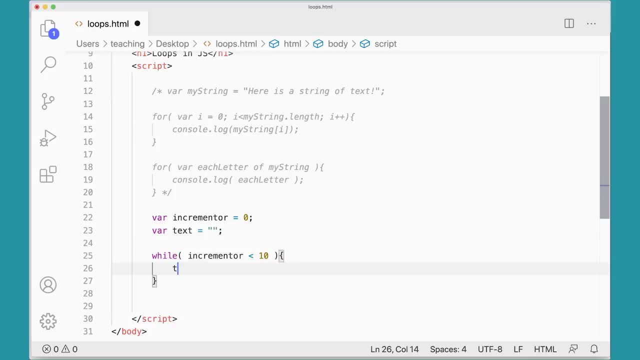 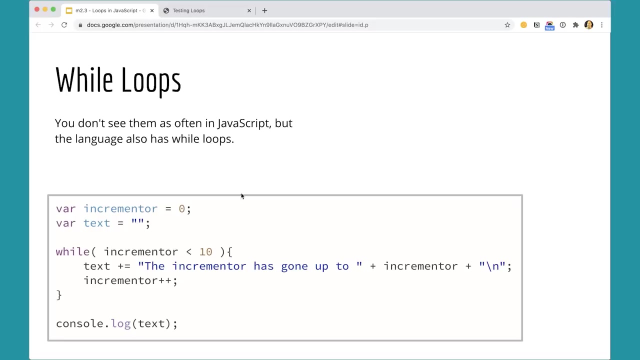 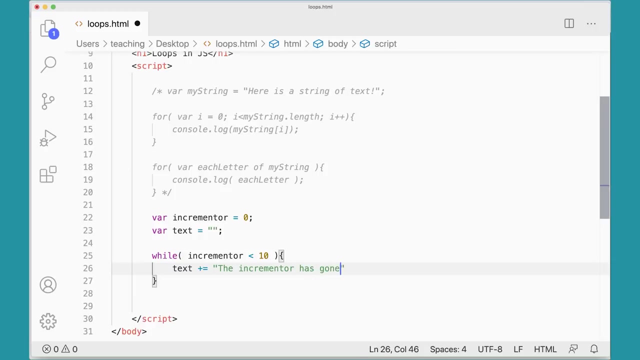 and what i'm going to do is i'm going to say: text equals, add to what was already there. quote the incrementor, incrementor. what did i put over here? i forget. now has gone up too. that's right. has gone up to. and then i need to add: 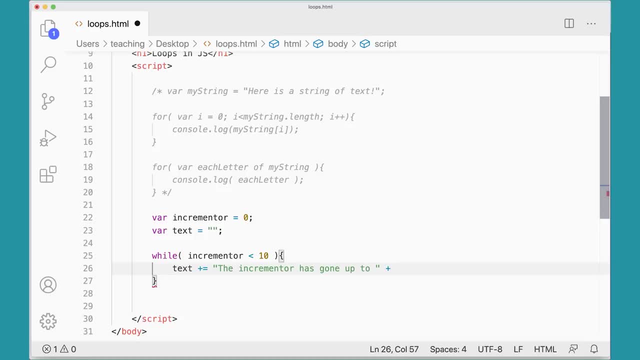 have a space there and i'm going to use a plus to concatenate in the incrementer variable. so it's gone up to whatever that number is, and then i'm going to add a plus and a and another set of quotes and now i need to add the new line. in this case i: 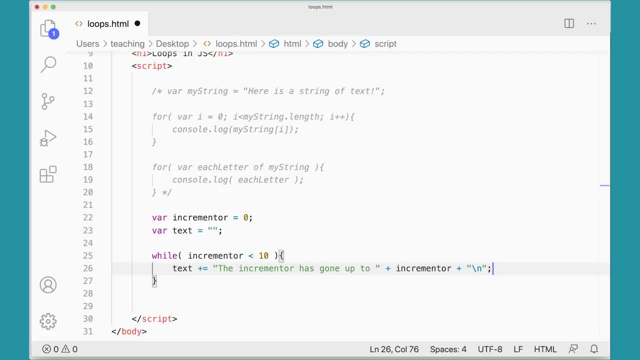 actually need the new line, because this is not going to get printed out. it's only going to get printed out once after the loop is done: incrementer plus, plus, and then down here i'm going to print the console log once with all the text in it. 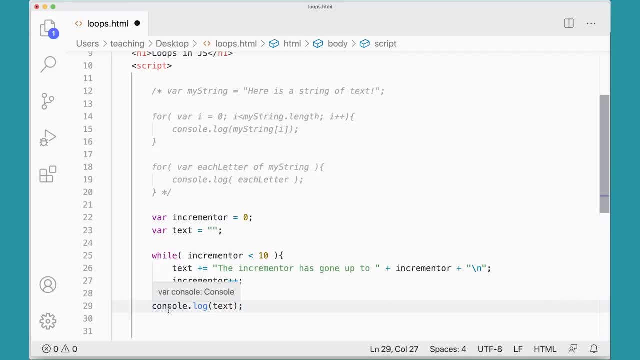 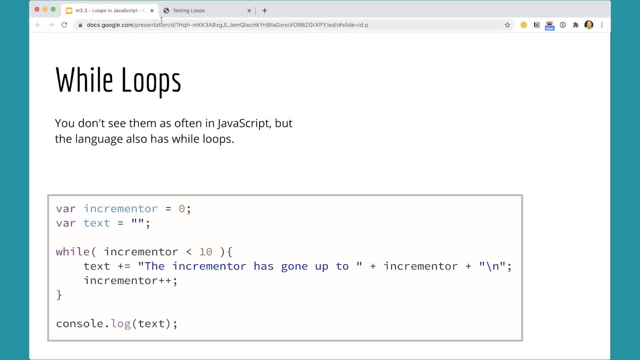 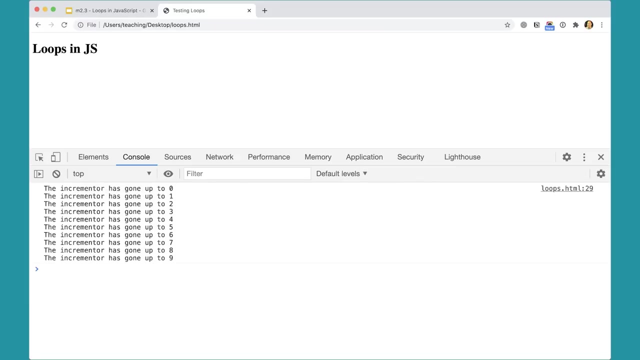 so there's one sort of print to the console log. all right, let's give that a try. if i didn't mess anything up here, let's see. and there we go. zero one, two, three, four, five, six, seven, eight, nine, if i didn't put the slash in on the end here. 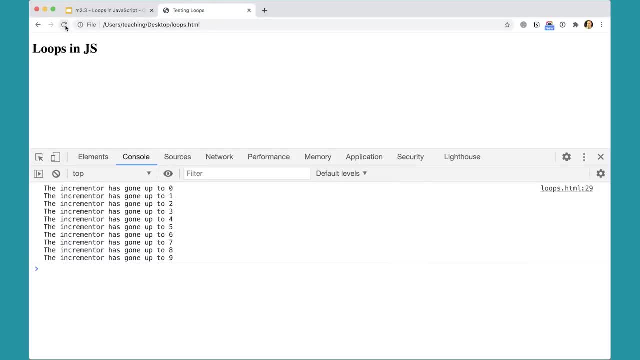 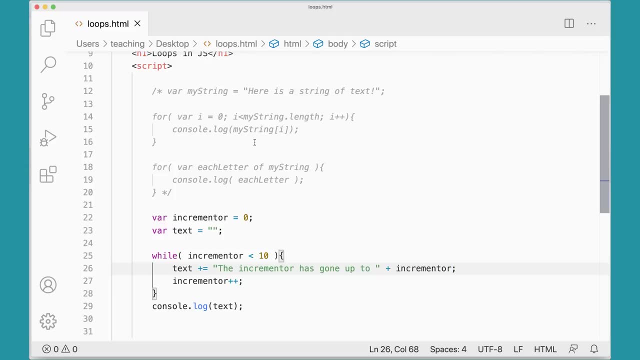 let's see if this does what i think it'll do, there we go. so i don't, i don't get the new lines, so the slash in is adding new lines over here after each one of these, because this is just getting printed at once. that's really kind of important to understand about the way this incremented. 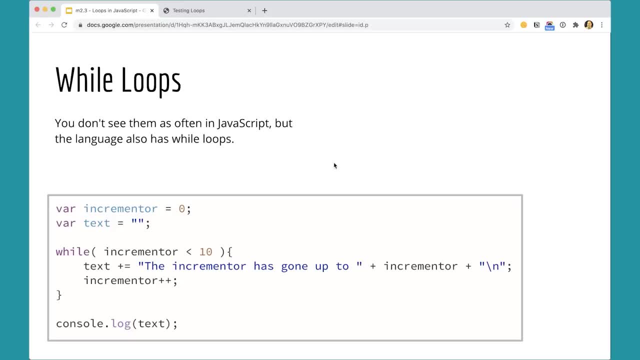 the way the while loop works here. when we look at this image here, we see that we have- we're using the plus sign to concatenate the string together with the variable, and we talked about this before. the plus sign in java's script does double duty. It's used to add numbers together the way you would normally. 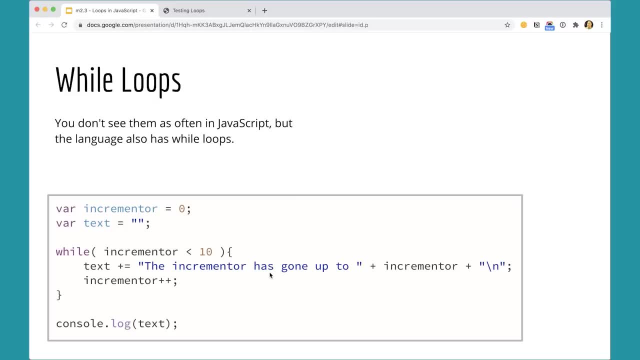 expect the plus sign to work, but it's also used to concatenate strings and things together. So here we've got a string of text and then we're concatenating in the variable and then another string of text concatenated on to the end of that And it gets kind of complicated to work this way. 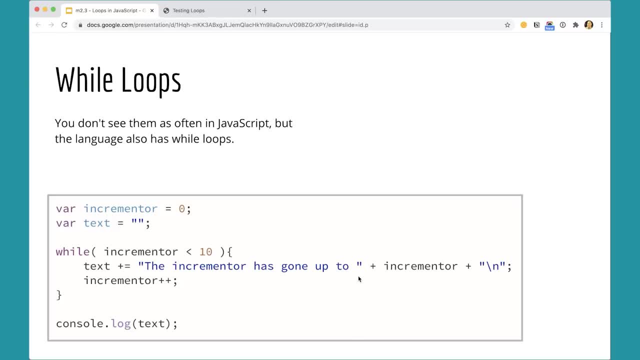 It's not very intuitive and we can't just leave incrementer inside the quotes, because then the string would just say: the incrementer has gone up to incrementer. JavaScript wouldn't know that this is a variable if we just put this inside the quotes. 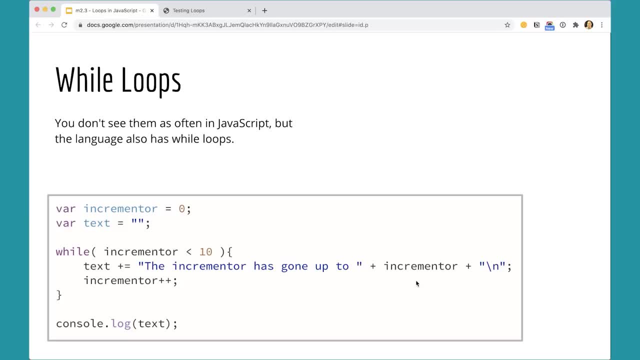 So with ES6, which, you remember, is the version of JavaScript that was released in 2015,- they introduced something called template literals that will allow us to work with variables inside strings a little bit more easily. So let's take a look at how to do that. 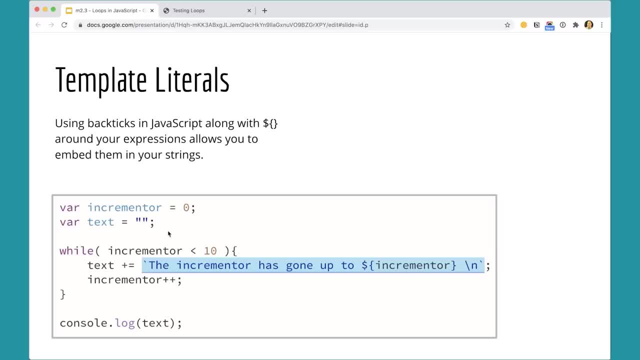 So here we have the template literal And with the template literal the way it works is we put a tick mark on either end. The tick mark is not a quote. The tick mark is a separate character in your keyboard. On the American keyboard it is the character with the tilde. 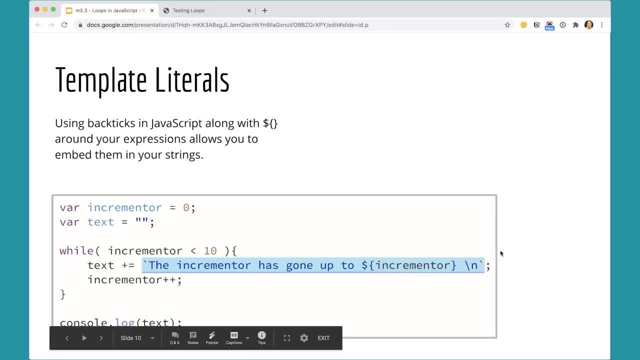 just above the tab key. So that's a tick mark there and a tick mark there, And then we can just put the variable inside curly braces with the dollar sign And JavaScript will know to treat that as a variable. So this is a much easier way. 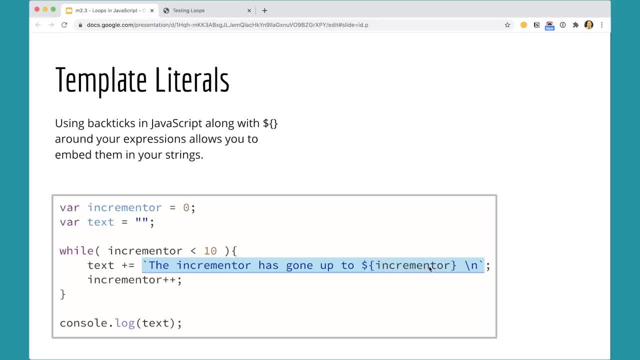 a much more readable way of working with strings with variables in them, And this particular string is not terribly complicated or complex in any way. But sometimes if you're constructing a piece of HTML and you've got tags, and tags have their attributes in them, which have quotes and equal signs, it can get really confusing really quickly. 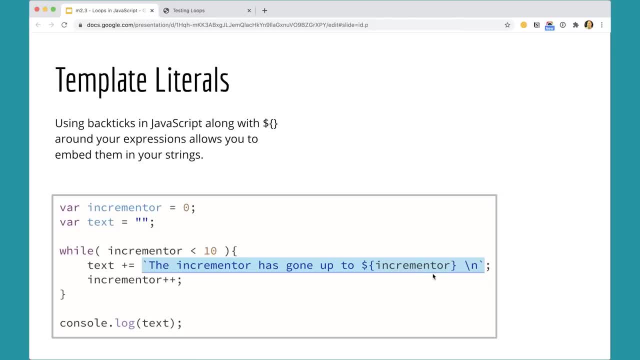 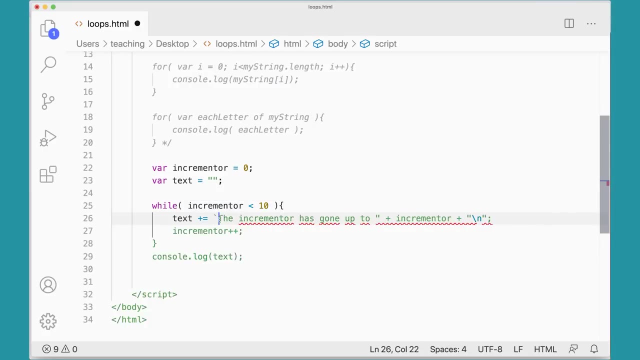 So this is: this will really help you out, And we'll be using the template literals throughout the rest of this course quite a lot, So let's switch our codes that we're using this over here. So the way I would do this is I'm going to put in a tick mark there And at the 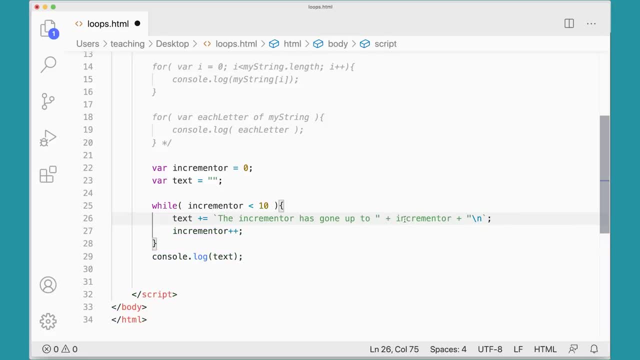 end, I'm going to put in a tick mark, And then I can get rid of these quotes and pluses, And then, because this is a variable, I'm going to put a dollar sign, a curly brace and another curly brace. And, by the way, if you're constructing a string that has variables, 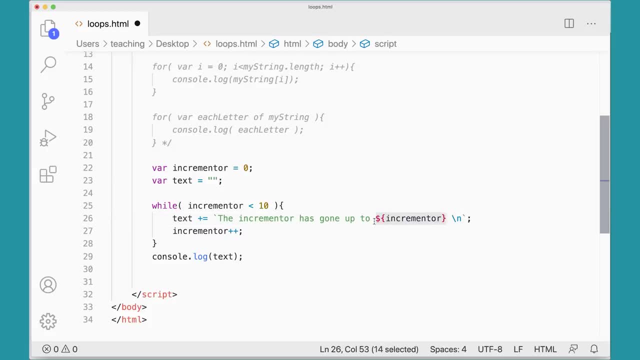 this is how I recommend that you do it, Rather than just typing from left to right. type it like this: The incrementer has gone up to incrementer, And then go in and add the dollar sign and the curly braces. You'll find it easier to understand what you're doing and to 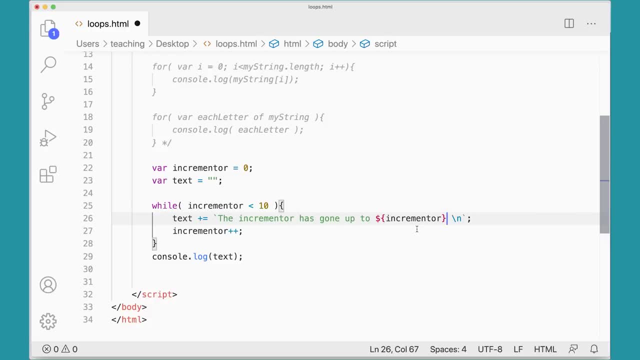 not make mistakes and do all that kind of stuff if you do it this way. But you'll notice, if I do this and save it and then go back and run the page over here, that I mean I just ran it, but it looks exactly the same. 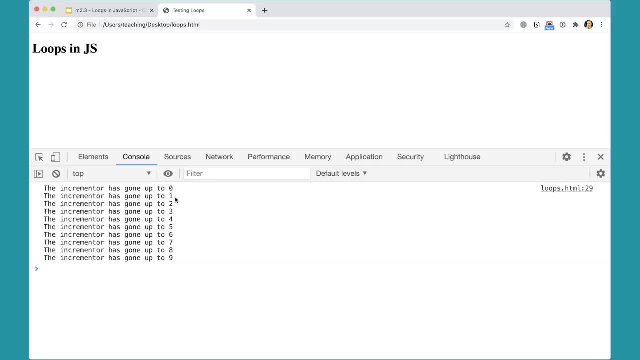 And I am getting my variables over here, So that really seems like a lot, of course, But they're very simple. So if you've just put in, so that is actually working. um, if you wanted to see if it was actually doing something different. 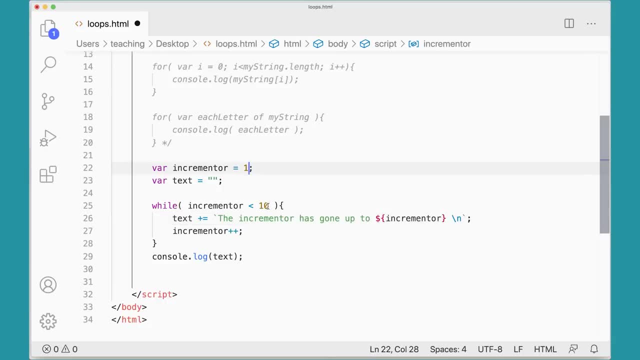 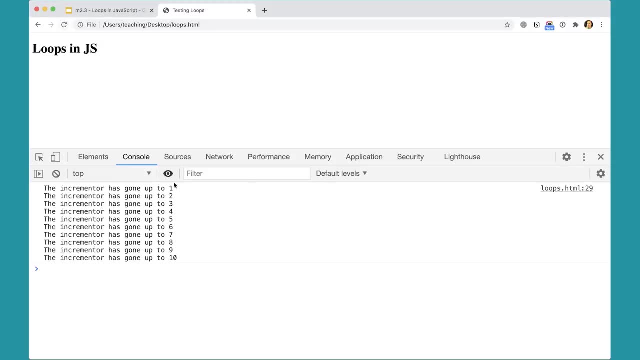 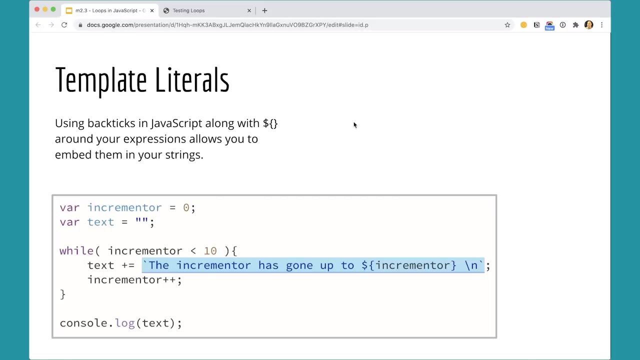 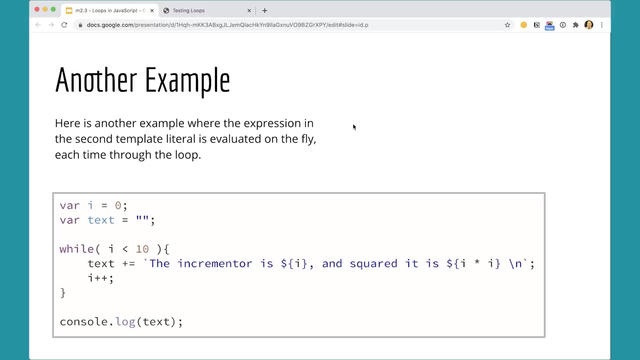 we could start here with one and go to eleven. see what that looks like. there we go one to ten. very nice, okay, so that's great. so we've got the template literals. that's really useful, and we're going to take a look at one more example. so what's kind of interesting here is we can: 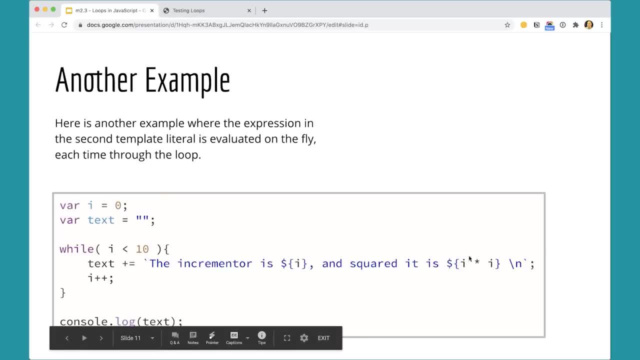 actually do expressions inside our curly braces here. so rather than just sticking the variable in there, we can actually perform javascript operations right in line with our string. so let's give this a try. and i set the incrementer to i to keep it shorter here, so let's do that. 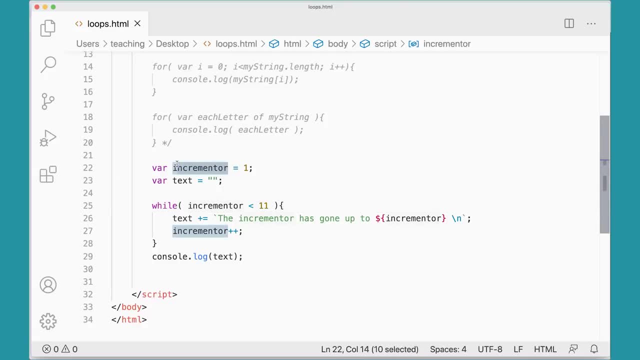 so whatever you here, i'm going to set this to just i. i is one. when we started at zero, i'm not sure we'll do one the incrementer, so do it like this: the incrementer is i and the incrementer square squared is i times i. but this is going to be. 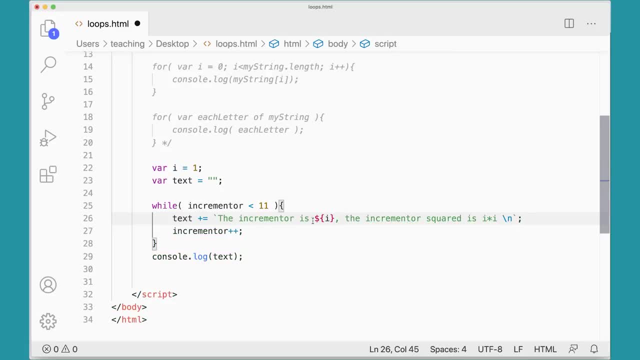 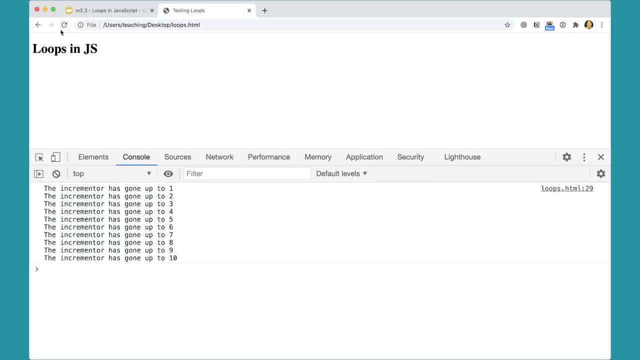 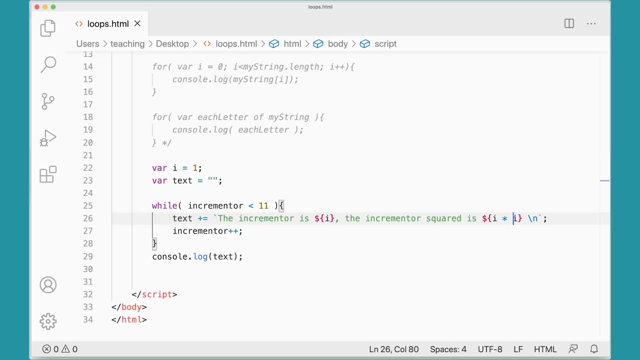 a variable, and so is this. it's going to be an expression. maybe i want some spaces there we go, so then we'll let that see. let's go see what that does. we go over here and run that. oops, incrementer is not defined. line 25: 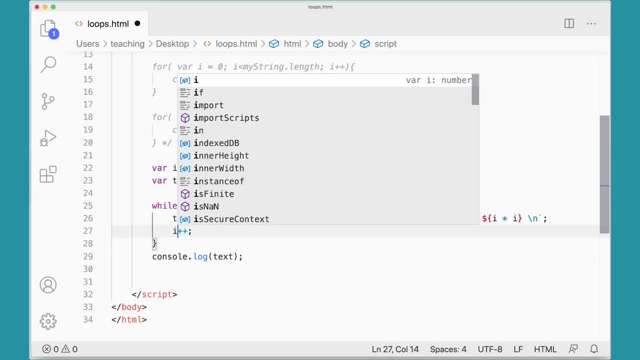 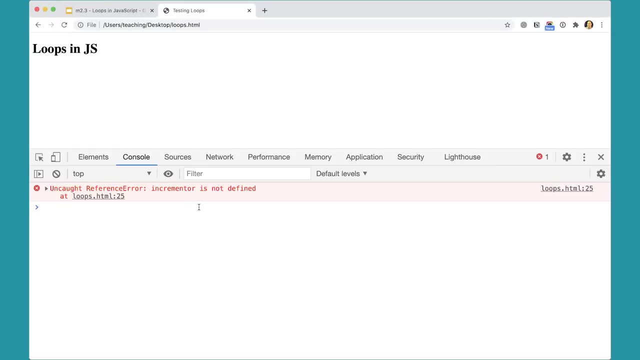 huge oh down here. that needs to be changed to i. that was a very typical mistake. it's great that these things come up while i'm doing this because you can kind of see how i fix them. so i could see right here. that was on line 25, i knew immediately. 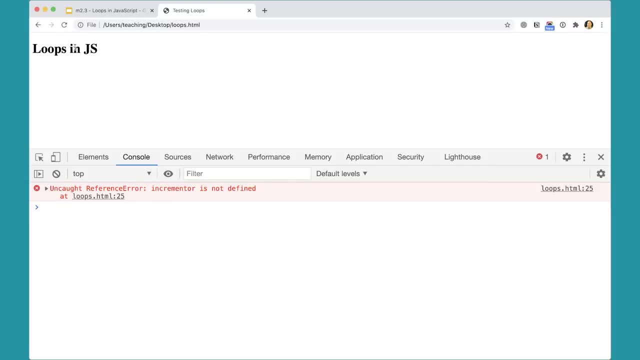 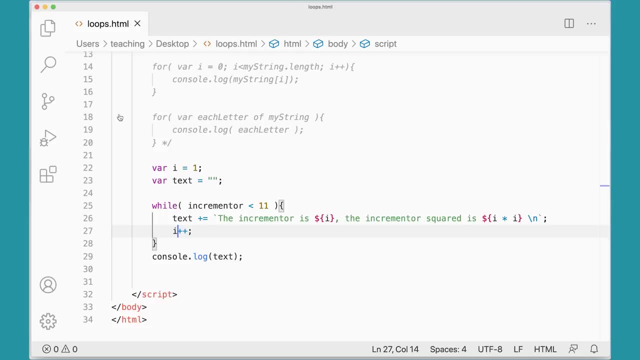 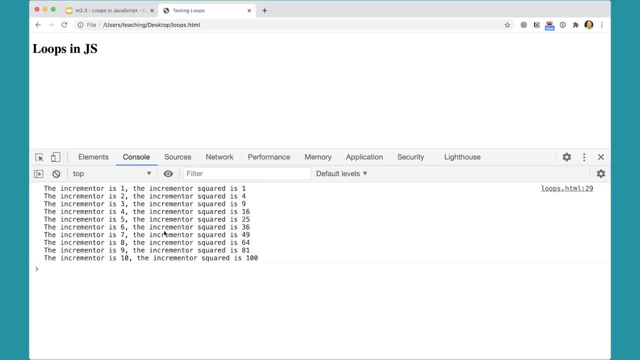 that i had forgotten to change an incrementer to. i just wasn't exactly sure where it was. but, and did i not save it over there? line 25: oh, this one here here also. there we go, and i'm getting my squares over here as well, so that's working great. 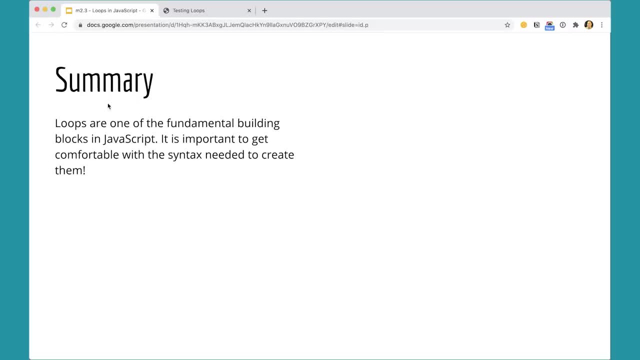 loops are one of the fundamental building blocks in javascript. it's important to get comfortable with the syntax needed to create them, and i recommend just sitting down and getting to the point where you can type in the syntax and you'll be able to get the syntax that you need to create. 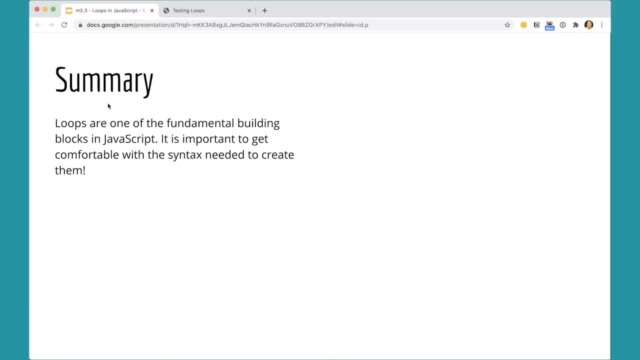 and type out a for loop. i know that it looks a little weird at first, but you have to just kind of keep working at it so you can get to the point where you could sit down and say, all right, i'm just going to write out a for loop, and when you get there then you'll know that you have. 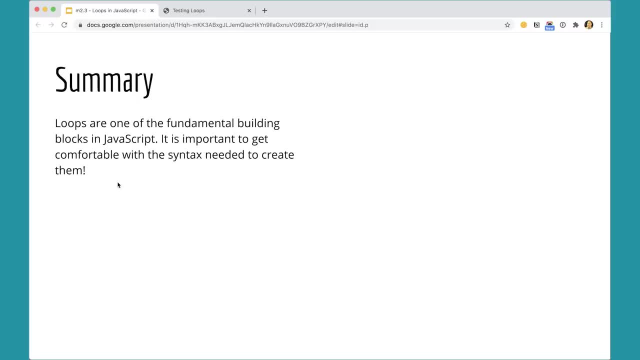 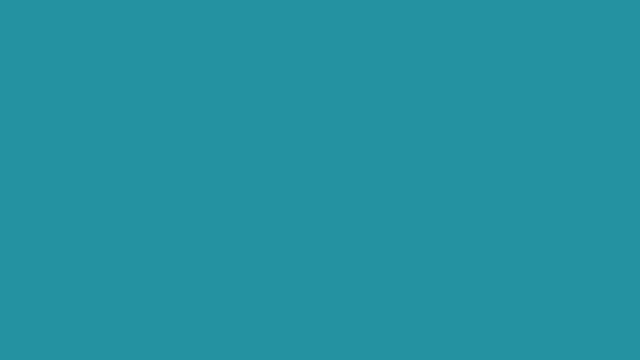 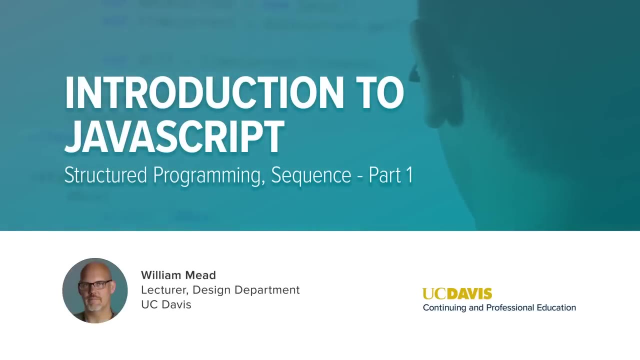 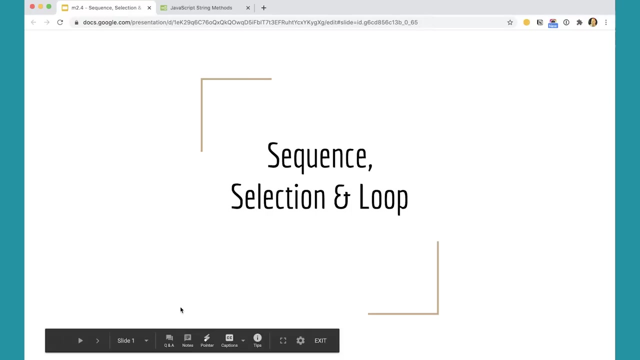 the loops really uh, down pat. okay, great, we're going to move on to the next thing: sequence selection loop. in this lesson we're going to put together some of what you've already learned and what you've already been doing and see if we can make some sense out of it. 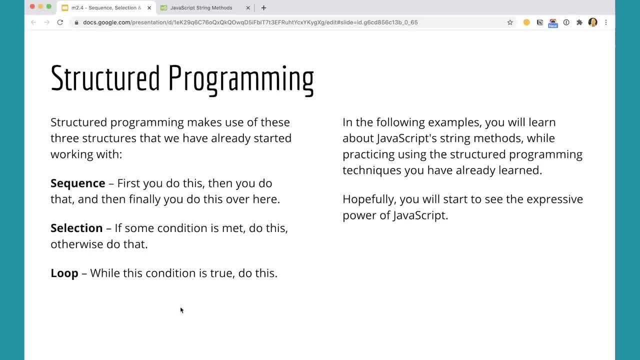 in structured programming we make use of these three structures. we've already started working with sequence. first you do this, then you do that. finally you do this over here with javascript. you start at the top of the script and you work your way down the script, and this is where i look for the 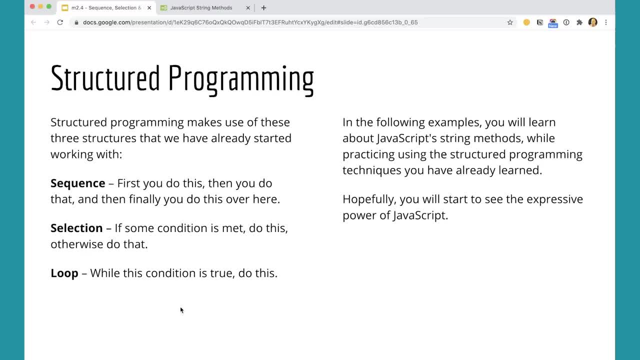 JavaScript does everything in the script, one thing at a time, in a sequence, With selections. we're checking to see if some condition is met. If this is true, do this, Otherwise, do that, And then, with loops, while a condition is true, we're going to continue to do something. 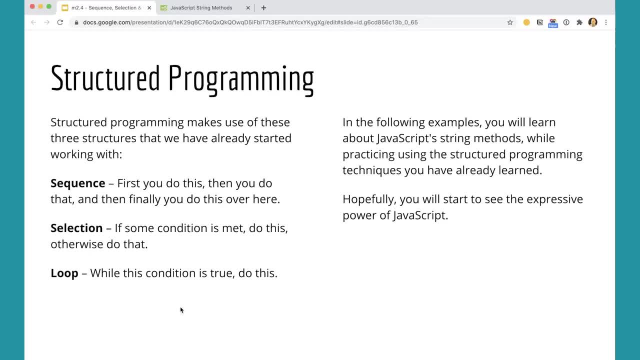 So with the scripts that we have next, we're going to learn a little bit about JavaScript string methods, while also practicing some of these techniques you've already learned a little bit about with loops and selections and these kinds of things, And hopefully you'll start to see the expressive power of JavaScript. 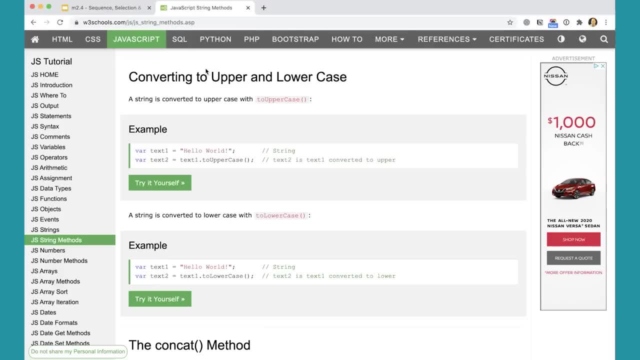 So over here I have some of the different string methods you can do, And to start with we're going to work with the toUppercase method here So we can actually take a string of text, assign it to a variable and then take that. 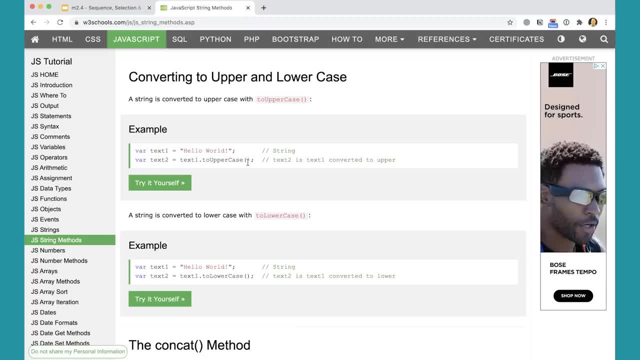 variable and do dot ToUppercase and that's a method that will take that string and convert it into an uppercase string, Or you can convert it to lowercase. So and if you come to this page you'll notice I'm further down the page here, but there's. 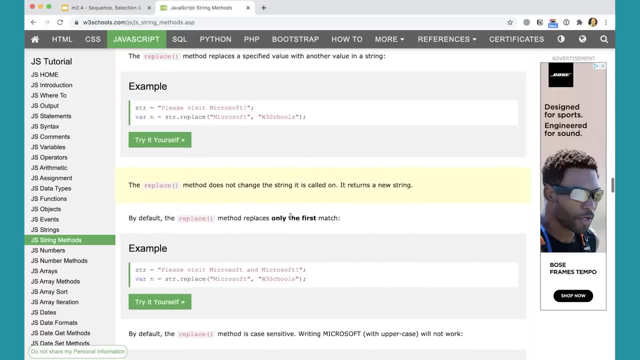 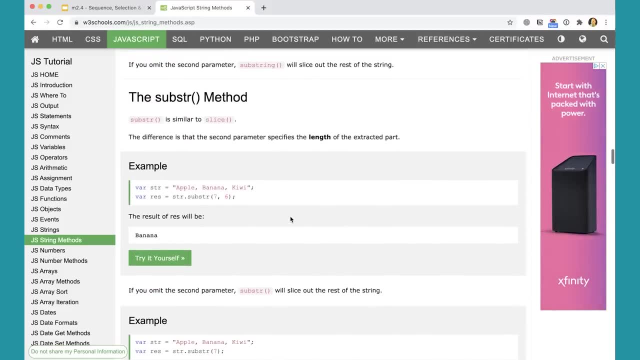 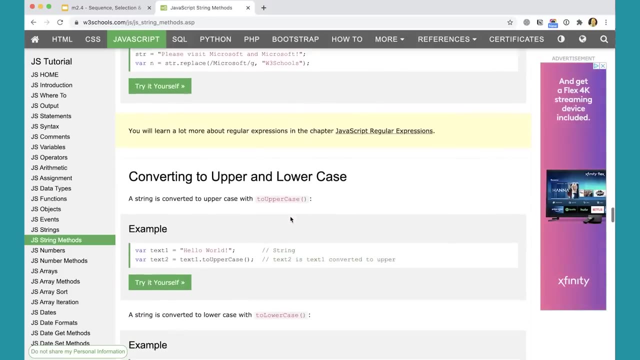 all kinds of different things we can do. to do with strings to replace content, to find content, to do all kinds of things with strings. We can take pieces of strings out of strings. We can perform string surgery. So this page is very useful for this kind of to explain some of the different kinds of things that we can do with strings of text. 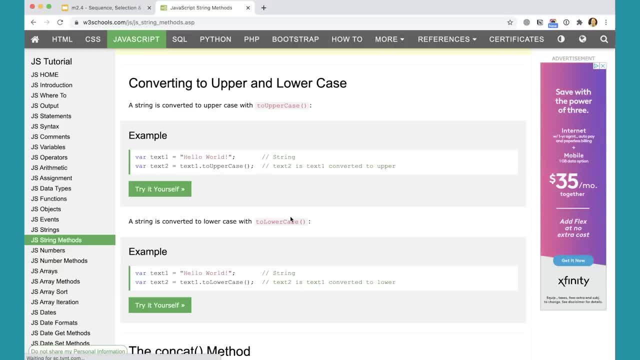 And you might be wondering: well, why would I want to do anything with a string of text, Why would I want to do this kind of stuff? But if you think about it, a web page, from the very first character of the web page to the very last character of the web page, is nothing but a string of text. 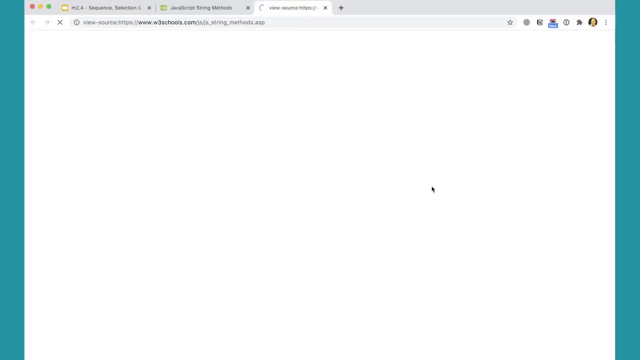 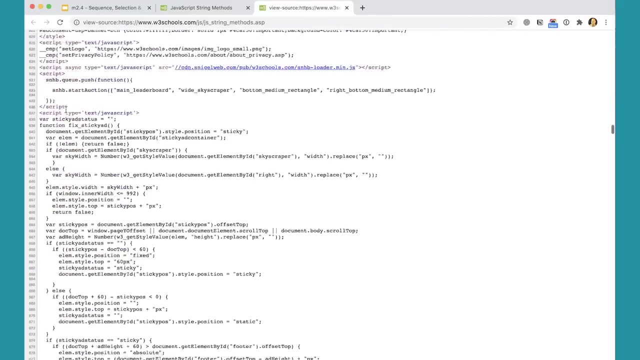 If I were to right click on this page and do page source, you can see it starts with a character And down at the bottom way, way down at the bottom, it ends with a character. This is one long string of text. 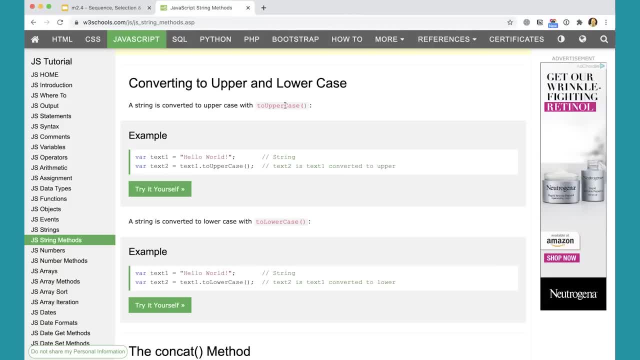 So in that, from that perspective, every web page is really just a string. So if we can do things with strings, we can affect web pages. Not that we're going to do it that way very often, but you actually can do it that way, which is pretty cool. 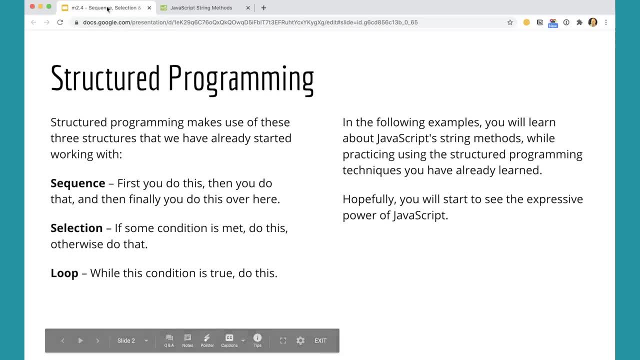 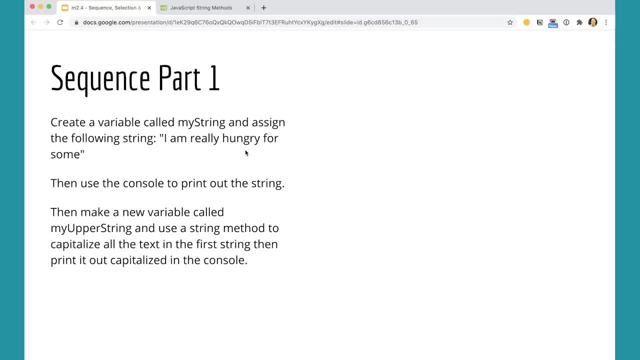 OK. so let's go forward with this and see what we're doing Here. So the first thing we're going to do is create a variable called my string and assign it the following string- I'm really hungry for some- and then use the console log to print out that string. then make a new variable called my upper string and use a method. 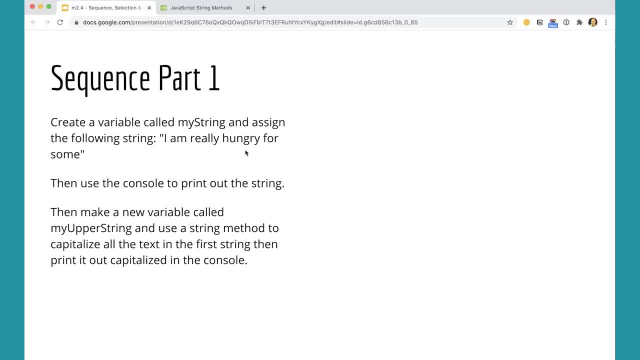 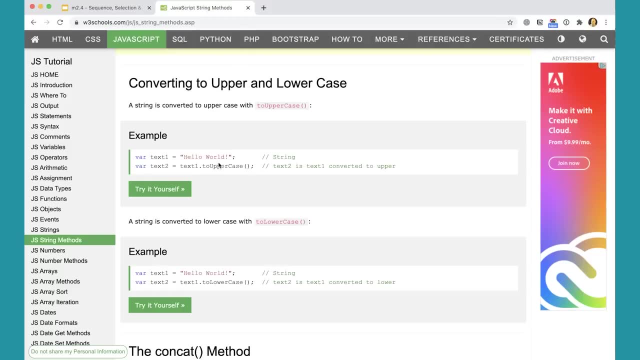 Use the string method to capitalize all the text in the first string and then print out the capitalized version of the console. Can you do that on your own? Try to do it using this two uppercase string method here And you can pause the video and come back and see how I did it. 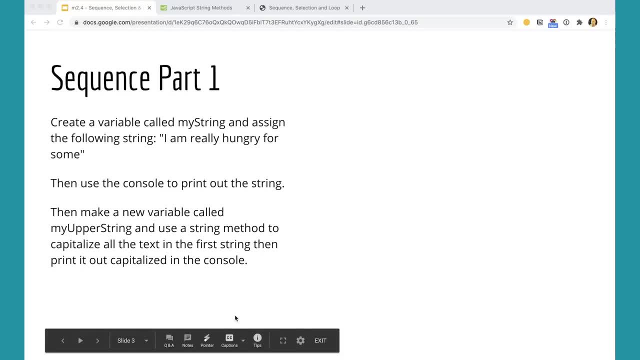 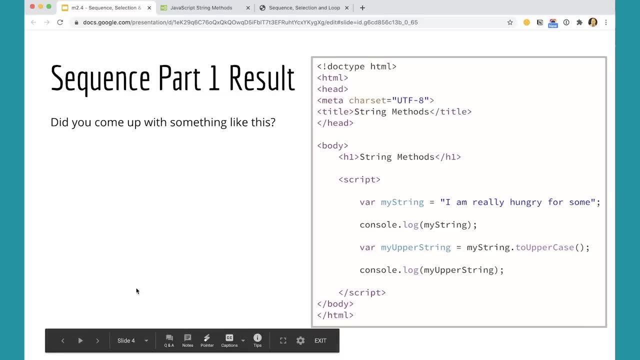 When you're ready, unpause the video and let's see if you have the same thing I got. Did you get something like this? I have it. I have the same thing over here in my visual studio code. I left out the spaces, but this is the same thing. 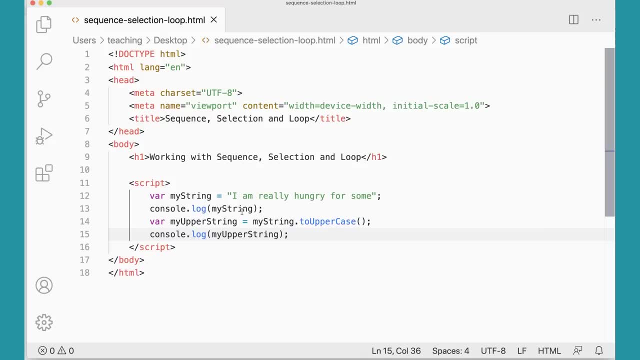 You're created a variable, my string assigned some text to it. I'm console Logging that out and make a new variable called my upper string, which is my string to uppercase, with the parentheses. This is a string method. We're going to talk about methods and functions and all that in a little bit, but for right now, understand that a method has these parentheses at the end. 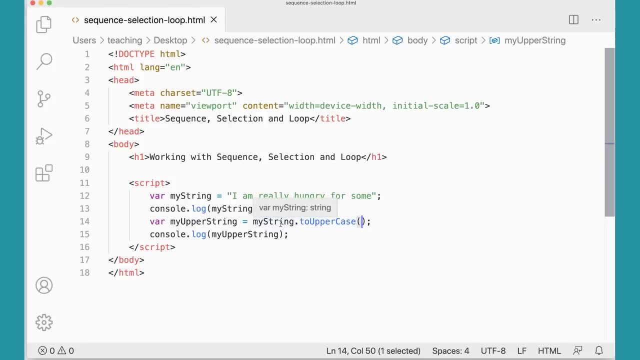 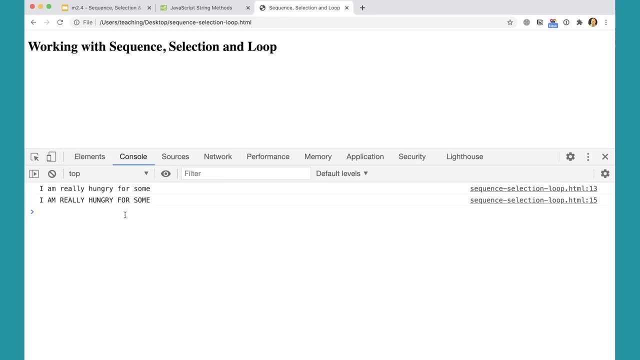 So um, and it'll, it'll take my string and convert it into uppercase and then I can console log that out and sign it to this and console log that out. So that works really great And I can come over here and see that actually runs and I've got both of my strings. 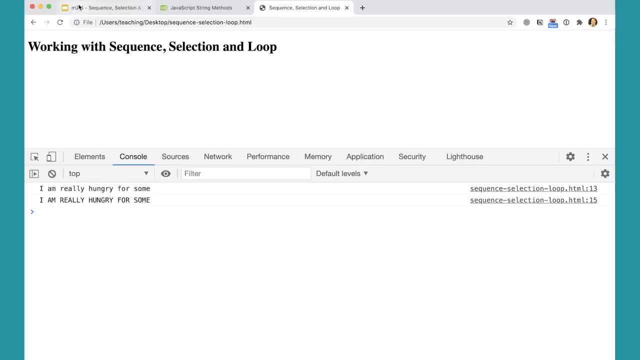 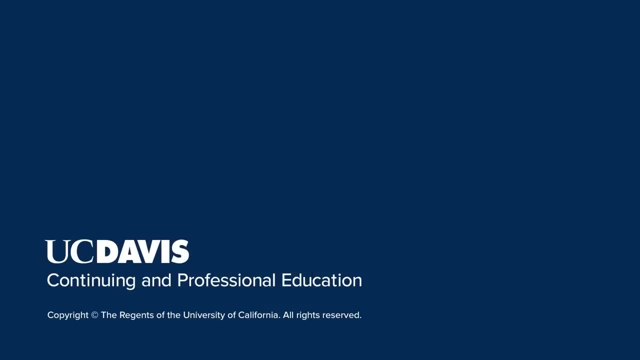 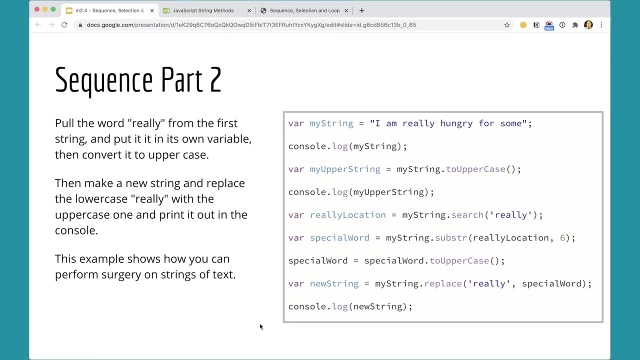 One of them is lowercase and one of them is uppercase. Okay, So that works great. Uh, let's see. what should we do next? Next, we'll do some more surgery on our strings. What we're going to do First here is we're going to pull out the word, really. 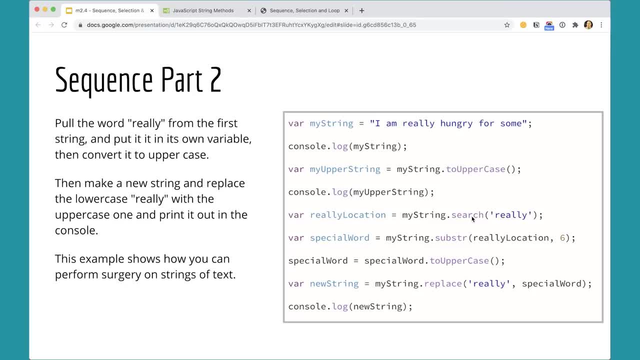 So I'm going to make a variable called really location and I'm going to use the search method to find out where this word really in my string starts. So what this is going to return is a number of that location. So let's do that first. 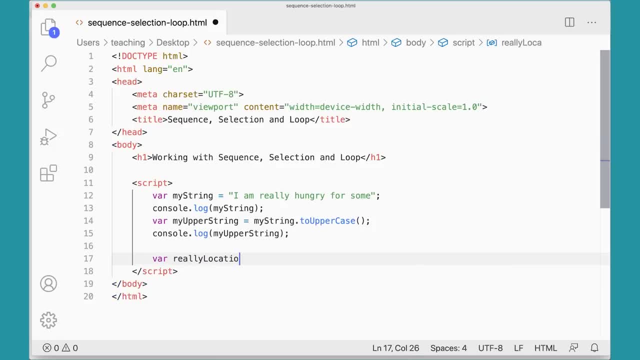 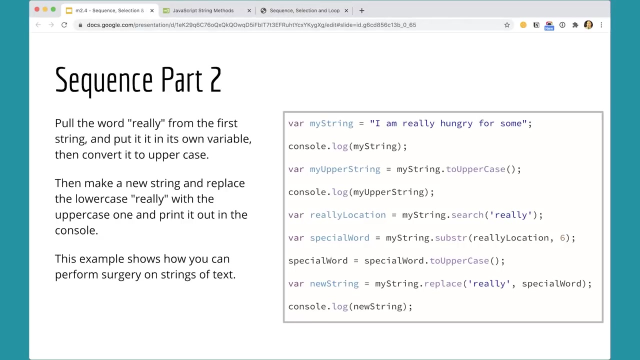 Bar really location Equals My string Dot search Really And then I'm just going to console log out Really location, Just so you can see exactly what that's getting. Assuming I did that right, I think I did. So that's getting a five. 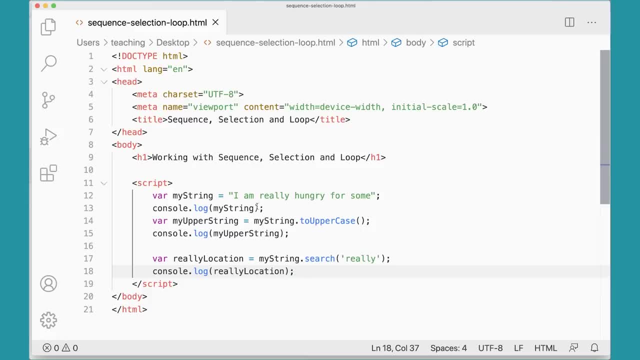 So what that means is that, If I count from here, zero, one, two, three, four, five- This is character number five. It's starting at a five. How many characters do I want to get? I'm going to get six characters. 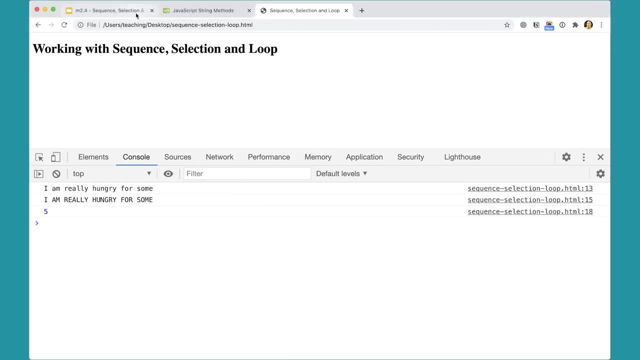 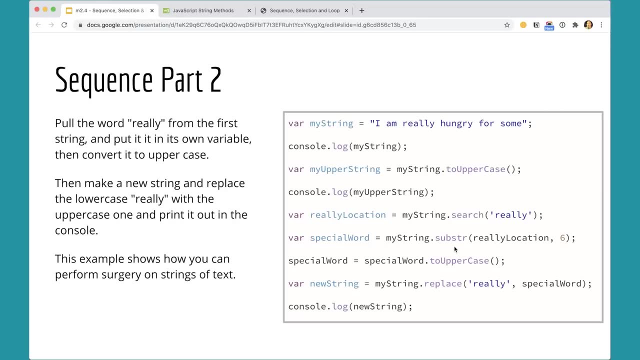 So I'm going to use The sub string function or or method here and I'm going to pass in really location, which is location five, and I'm going to get six characters, And what that's going to do is it's going to pull out into this variable special word the word really. 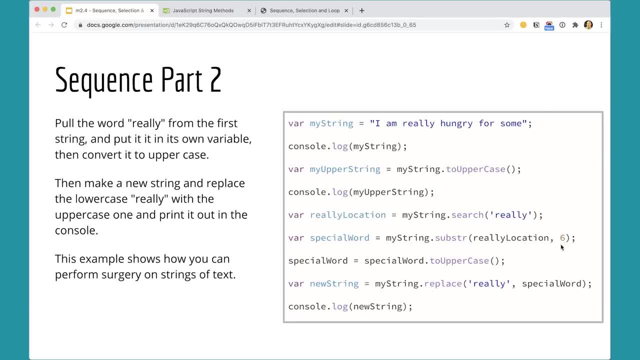 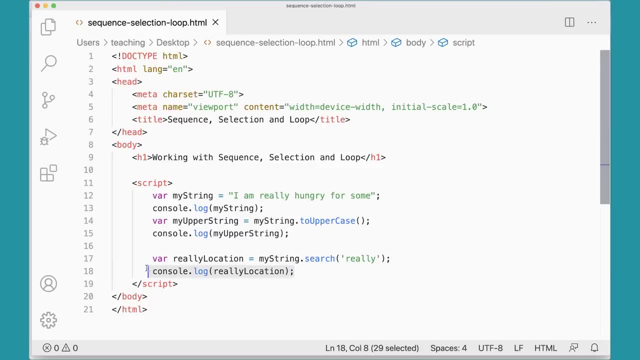 It's going to start at five from my string and get six characters. So let's do that. Bar special word equals string, dot, sub string And I'm going to start with really location and get six characters And if I console log Special word. 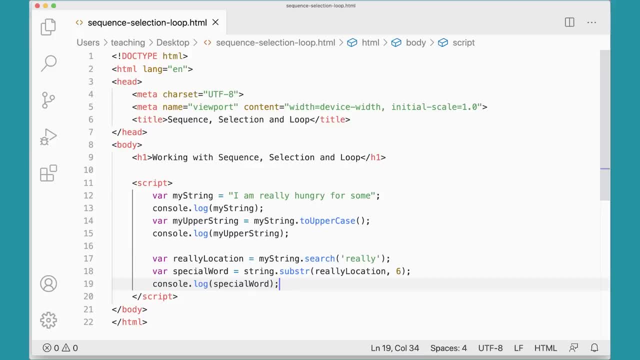 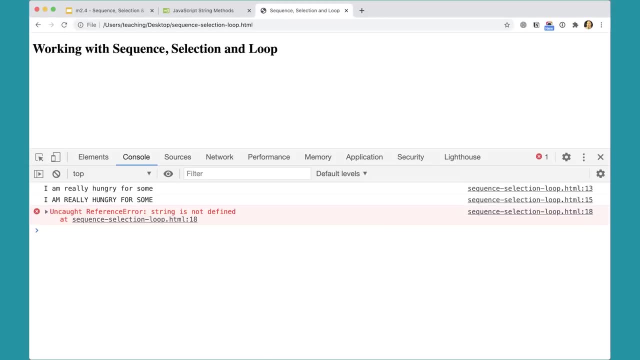 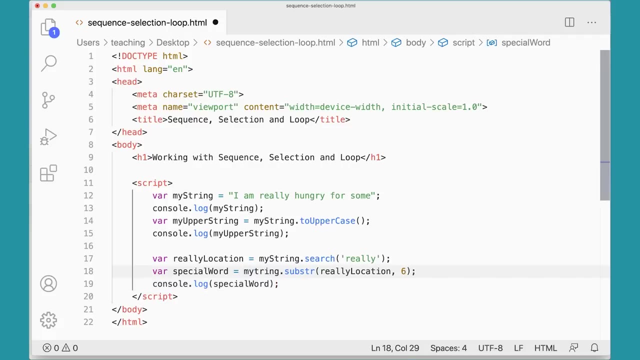 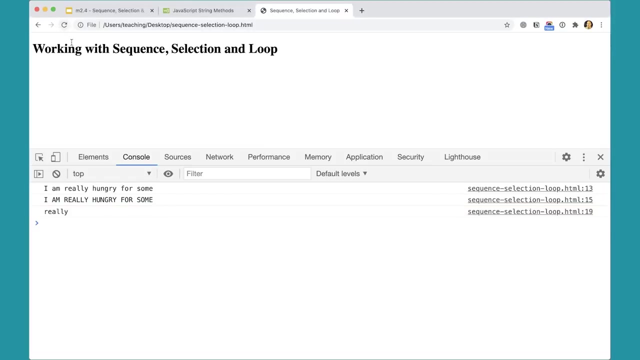 You'll see So what that's getting for me. Oops, I misspelled. Oh it's. it's my string, isn't it My string? With a capital S. There we go, There we go. Now I'm getting the word. 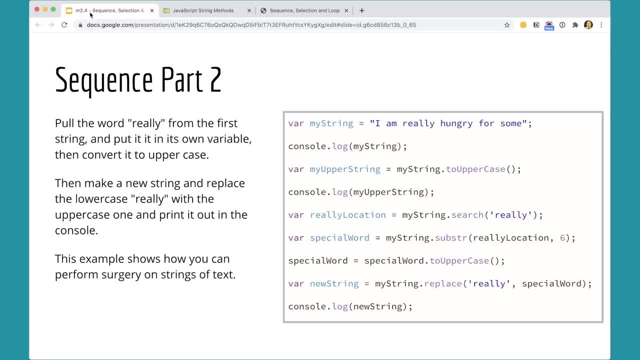 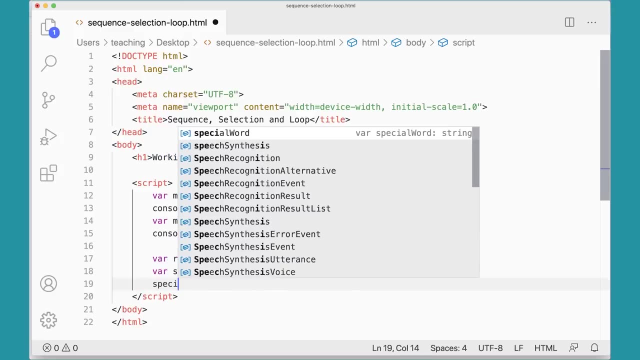 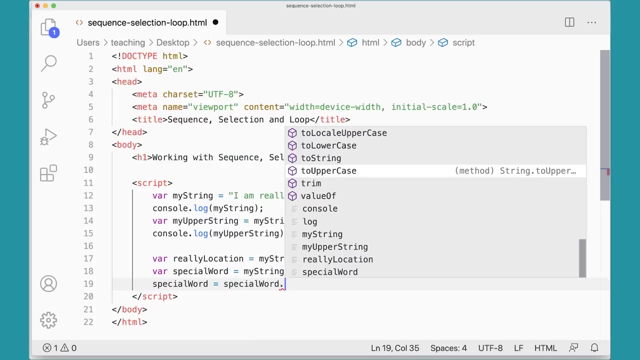 Really great. So I've got that. now I'm going to take special word and I'm going to sign it back to itself, but uppercase. So I'm going to say special word, I'm going to assign it special word: dot two uppercase. 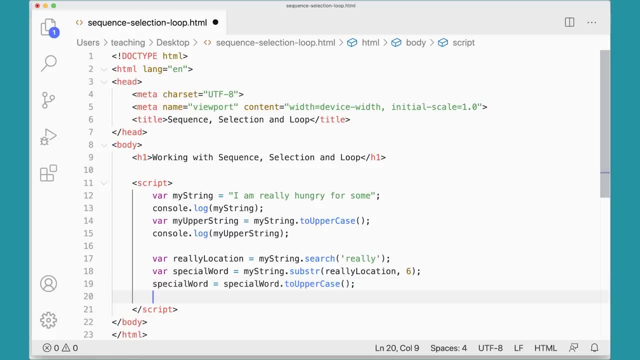 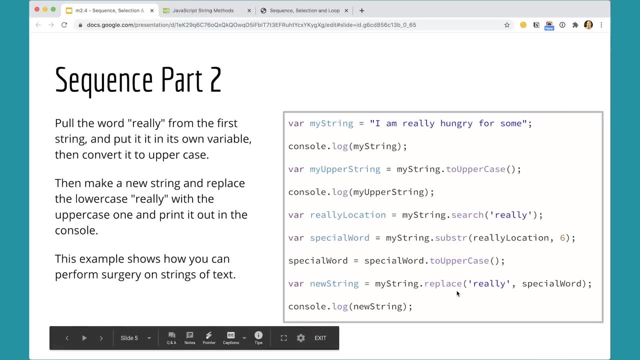 So now it's going to be uppercase and and then what I'm going to do is I'm going to make a new string and I'm going to replace, really with special word into the original mice my string here and then I'll console log out new string. 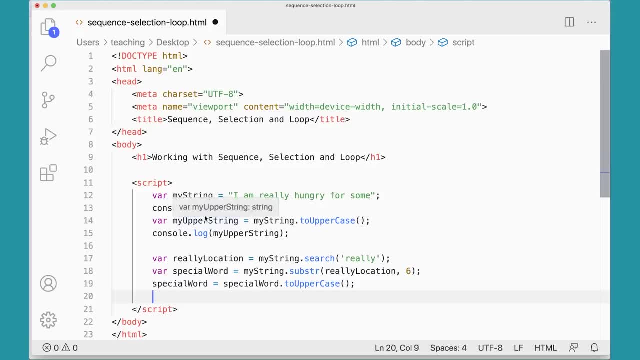 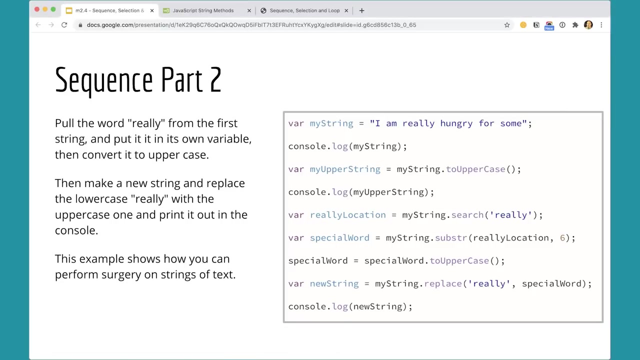 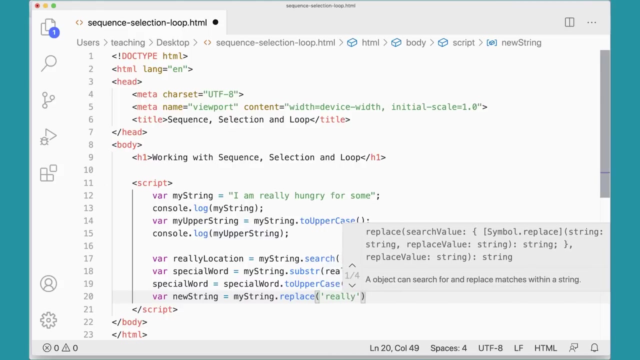 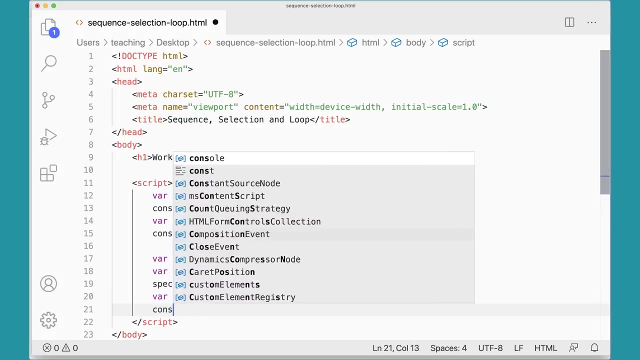 So let's do that. Bar new string Equals my string. Dot replace. And which order does it go in? I'm going to replace really with special word, Special word like so, And then I'll console console: dot log New string. 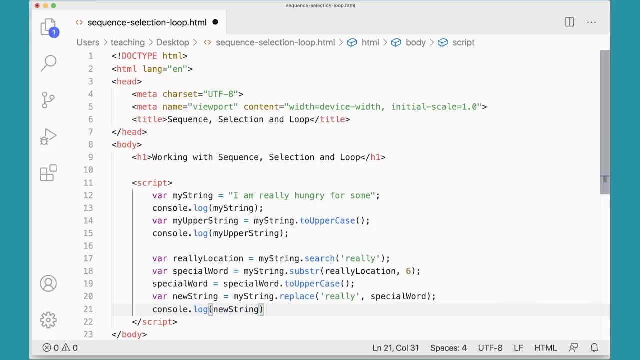 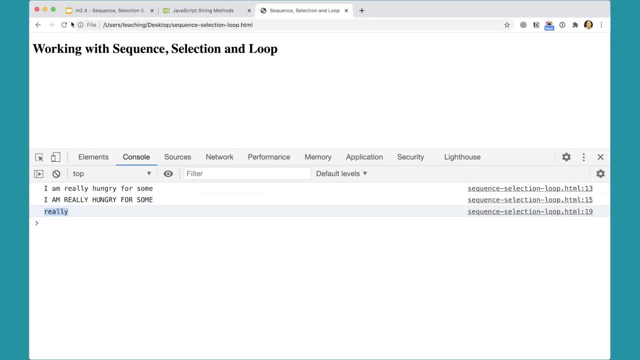 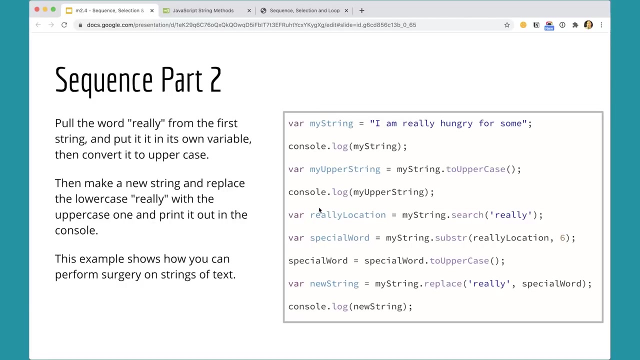 And what I should get is: I am really hungry for some. So I'm getting the capital word really there, And but this is a sequence. JavaScript is doing a sequence of things, One thing after another, after another, other after another. 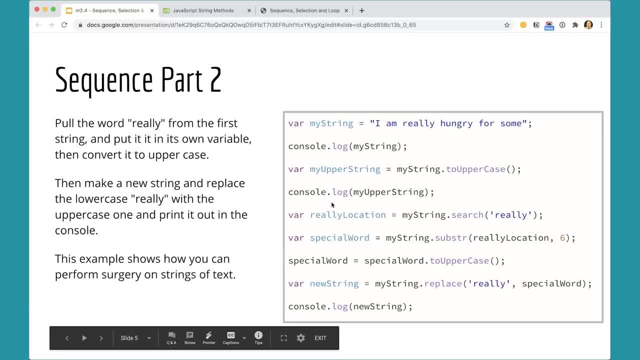 Which is a sequence. So I'm just doing a sequence of things here And JavaScript goes through the script one step at a time And we're just learning about some string methods along the way. We've learned about a few of them already. 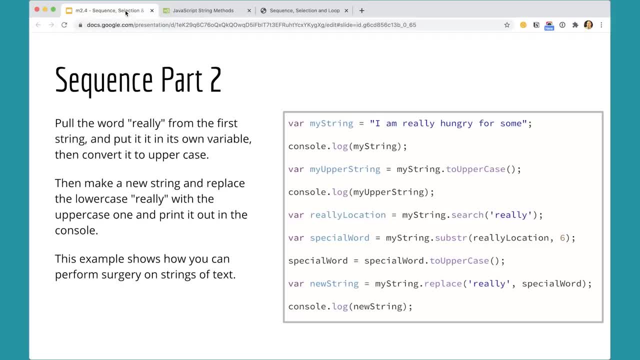 Uppercase and replace and search and substring, And there's a lot more here that you can go through and learn, But that'll get you started to begin with with the various string methods that are available in JavaScript. We're doing string search. 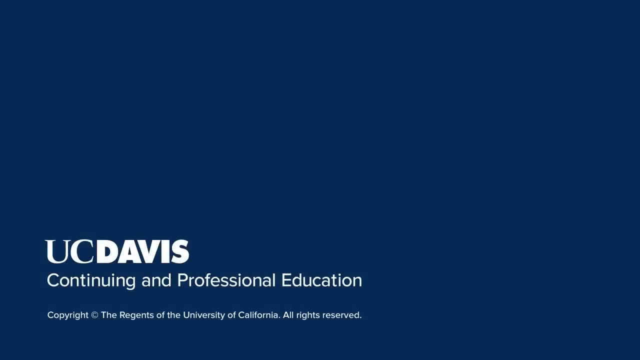 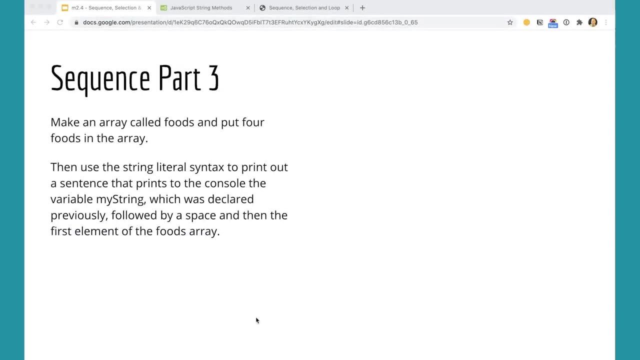 And I'm going to take a set of nonшей For the next step in our sequence. Make an array Called foods And put for foods in the array, Then follow that with a space and then the first element in the foods array. See if you can do. 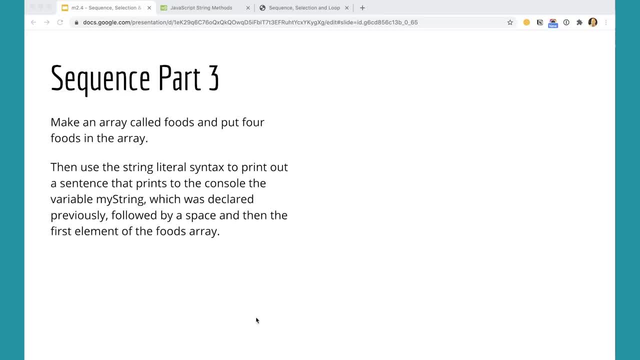 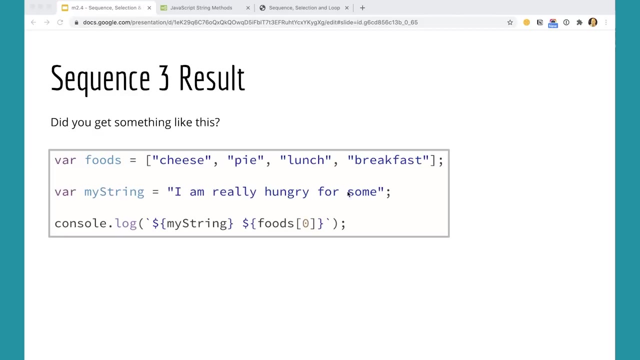 that. Pause the video and see if you can do that without looking at the answer that I have next, And when you're done, unpause the video and come back and we'll see how I did it. Did you get something like this? I have my string in here again, but you shouldn't need that, because 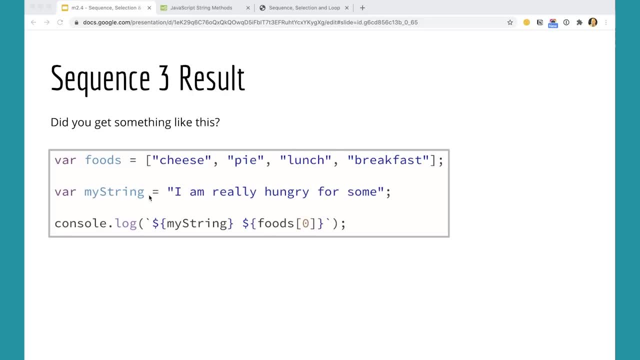 we already have that on our file. But you should have an array and then the console log with the template literal. It takes a little getting used to the template literal thing. Let's do that part together. So over here you can see I've added the array and then here I need to add the template. 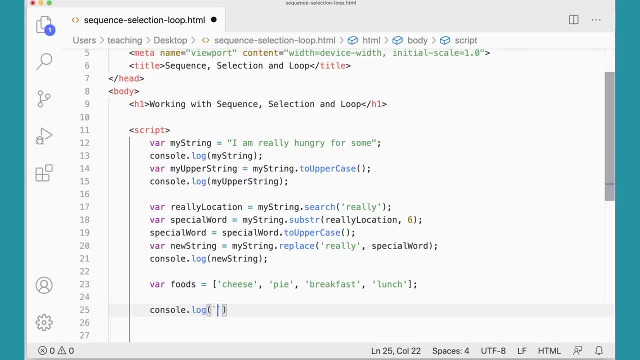 literal. So I'm going to do- and the way to do this, the best way to do this, is to just type the variables, my string, and then I want a space and I want foods, square brackets, 0.. But these are variables, so I'm going to come in here and add a dollar sign and a curly brace. 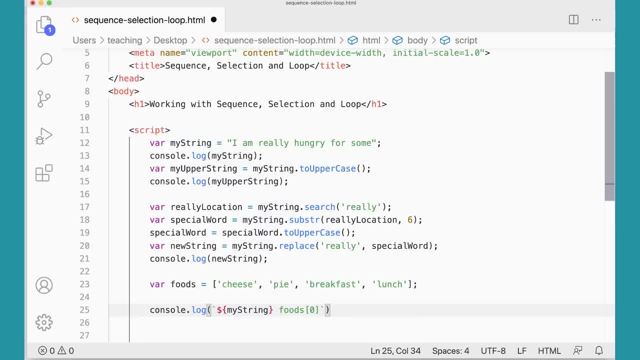 and a curly brace And then a dollar sign and a curly brace and a curly brace around it, And if you do it that way, you'll understand it better. if you always sort of work from the inside out or the outside in, In this case we're sort of working from the inside out, but if you work 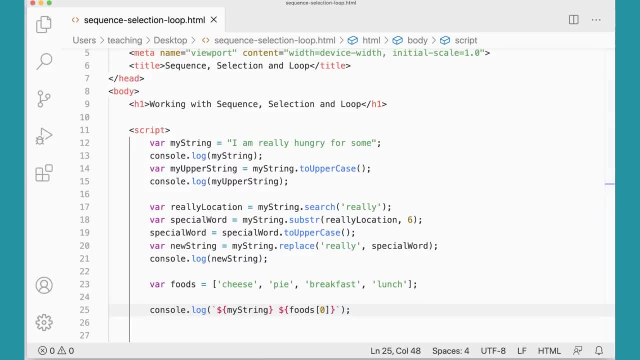 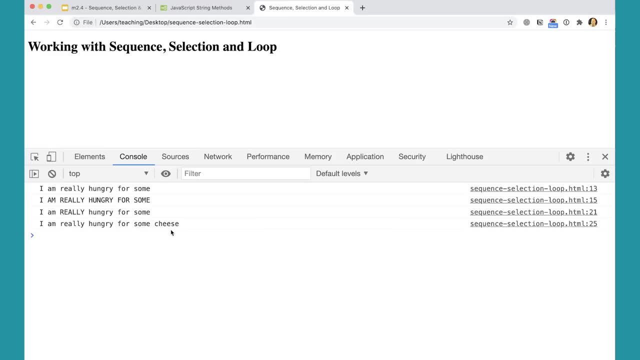 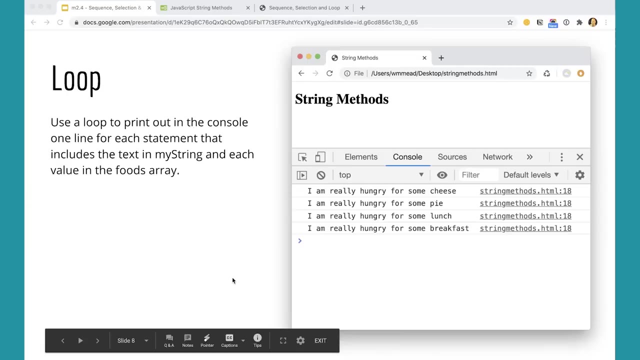 that way it'll make it easier for you to understand it. So I'm going to do that, And then over here I can actually run that and I should be getting. I'm really hungry for some cheese, So that works perfectly well. Okay, great. The next thing to do is to see if you can use a. 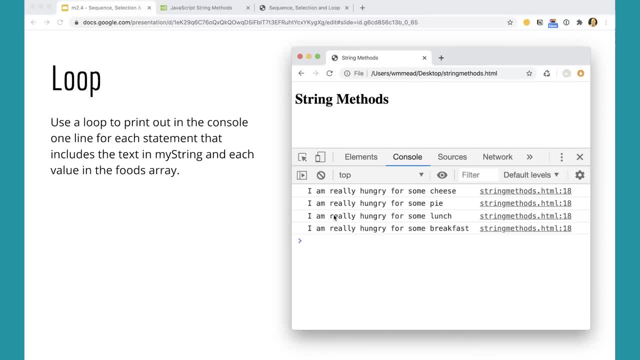 loop and loop through all of the elements in the array. I'm really hungry for some cheese, for some pie, for some lunch, for some breakfast, all of these elements. So let's see if we can do that. Go ahead and try it. See if you can write the loop. 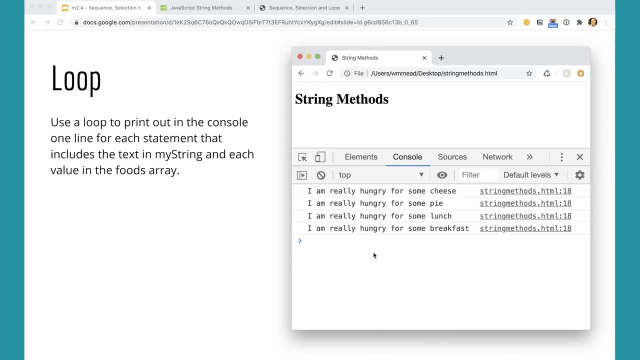 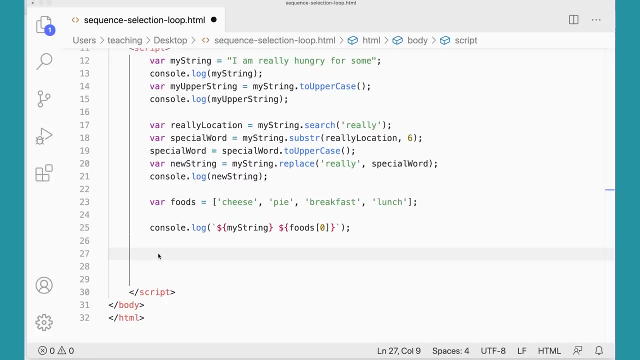 For yourself. pause the video again and see if you can write it. Try using the for loop, Try using the for of loop. See which one feels better to you. Try them both. Hopefully you got it for yourself, but I'm going to do it here, just so you can see how I do this. 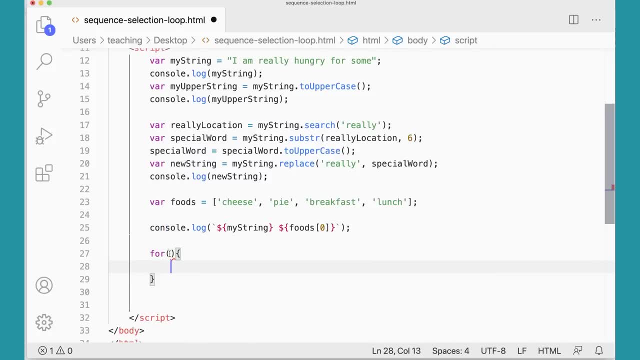 For. and then I'm going to come in here. I'm going to say bar i equals zero. I'm going to start at zero, While i is less than foods dot length. Now I could stick in here a four instead of foods dot length, but this is better practice. 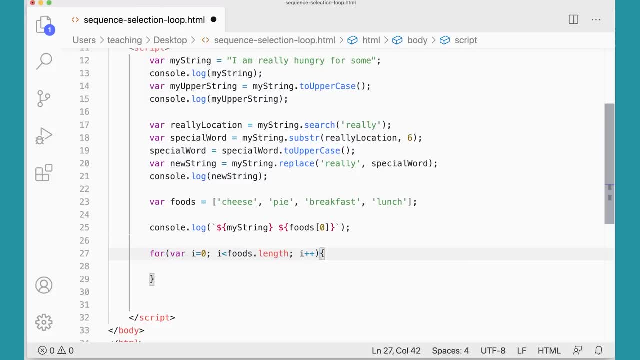 Foods dot length: i plus, plus. And then I'm going to console log out. basically this line here. I'm just going to stop, I'm going to stick that in there, but instead of food zero I'm going to put an i in there. 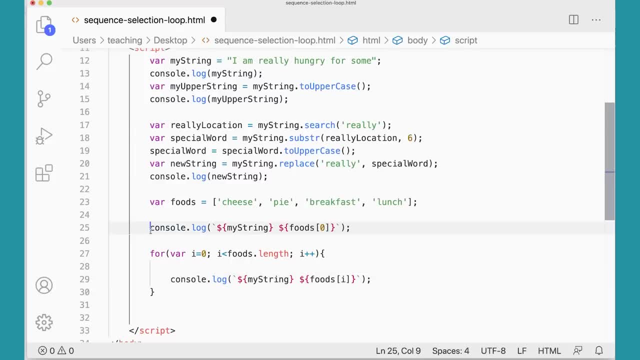 because I is going to get each one of these. In fact, just so I don't get confused, I'm going to comment that line out there, just so I can see this is really working. So first time through the loop, i is zero, So it's going to print out. 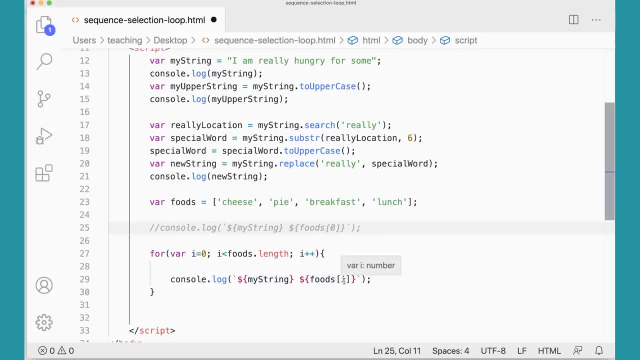 I'm really hungry for some space food. square bracket: zero: because i is zero, i gets incremented to one. So the second time, Second time through the loop, 1 is less than 4, because, remember, this is going to be a 4.. 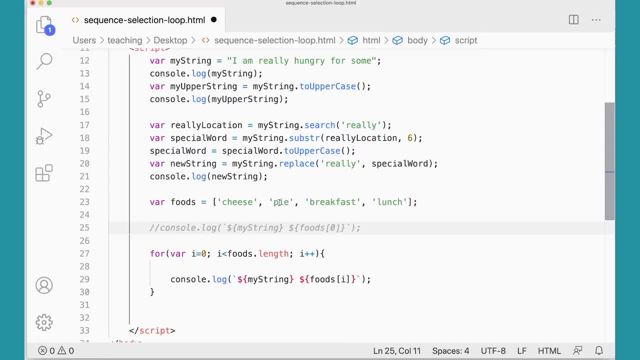 So it'll go through again and it'll get pi, And then the third time through the loop it's going to get breakfast, And the fourth time through the loop it's going to get lunch. And then i gets incremented to 4, because it's 0,, 1,, 2,, 3.. 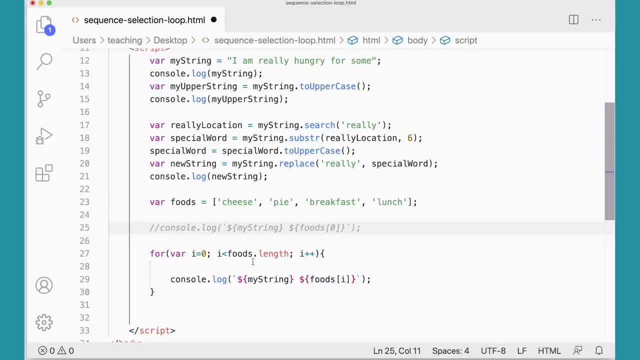 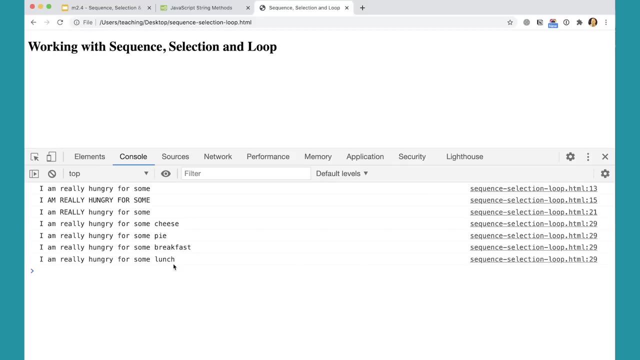 So i is going to get incremented to 4.. 4 is not less than 4. So the loop will bust out. Let's see if that works. And there we go. We're getting all of it there. That's great. 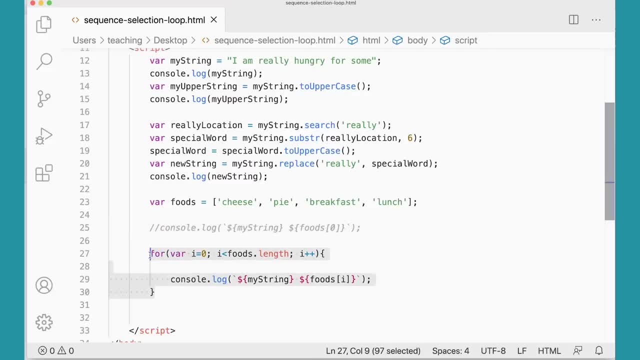 Now what if you wanted to use the for of loop? I'm going to just comment that out For var For each food of foods. Something like that will work. It doesn't have to be each food. You could do i if you wanted to. 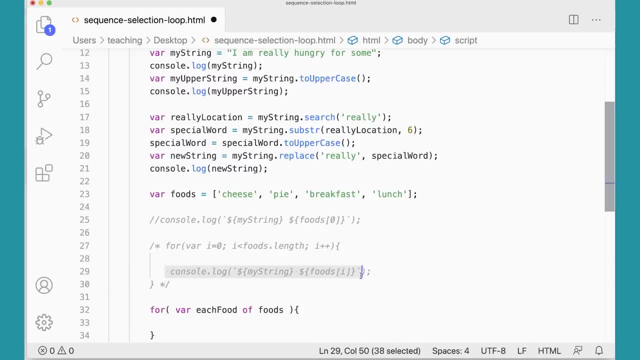 And then in here we're going to do the same thing. We're just going to basically take this and stick it here, But now, instead of foods, this food's i. this is going to be each food I'm still going to print out. 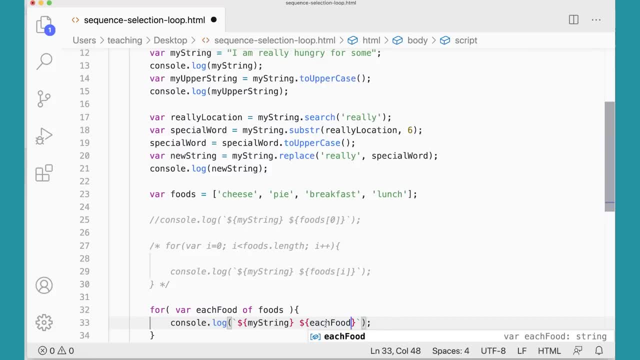 I'm going to print out. I've got my string, but now this is going to be each food. So the first time through the loop, each food is going to be cheese, and then the second time through the loop it's going to be pie, and then it's going to be breakfast, and then 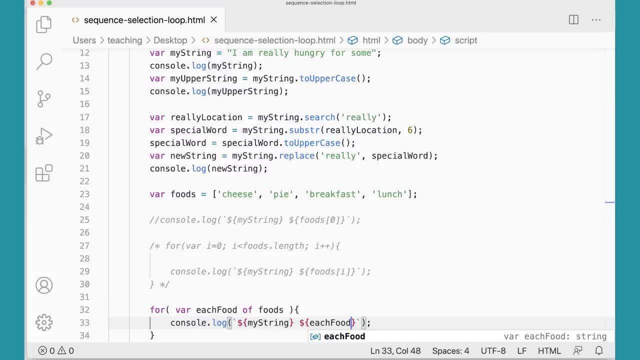 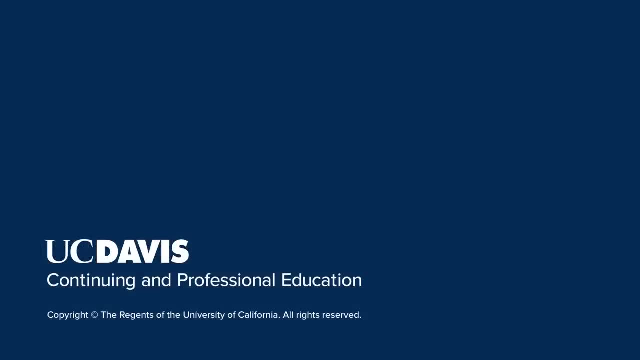 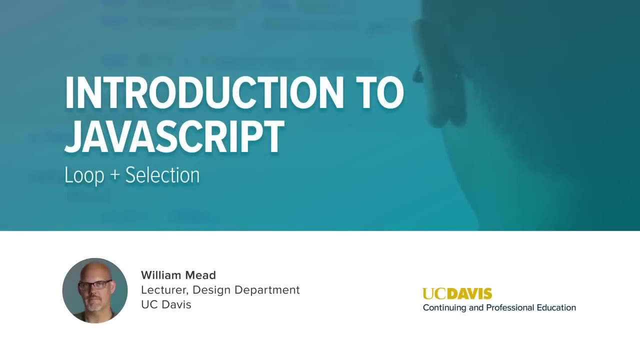 it's going to be lunch and we should get exactly the same results, So it's going to test it out to be sure, And sure enough, I get the same results. Next, we'll bring selection. Next, we'll bring selection. 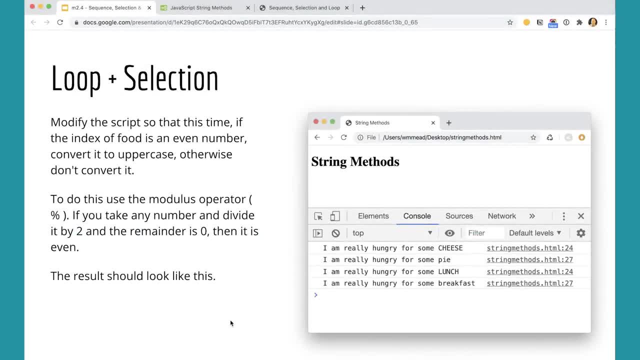 Next we'll bring selection. So now, inside our loop, we're going to check to see if the element in the loop is even or odd, And if it's even, we're going to make the word for the food that we're getting out of the array all uppercase. 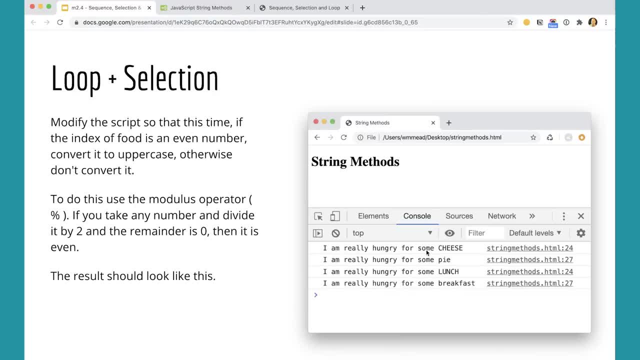 like this over here. This should be your results. I'm hungry for some cheese- all capital letters there- And I'm hungry for some pie, and that one's normal. And then lunch Lunch is going to be uppercase. Now you might be wondering: well, wait a minute, that's not even. 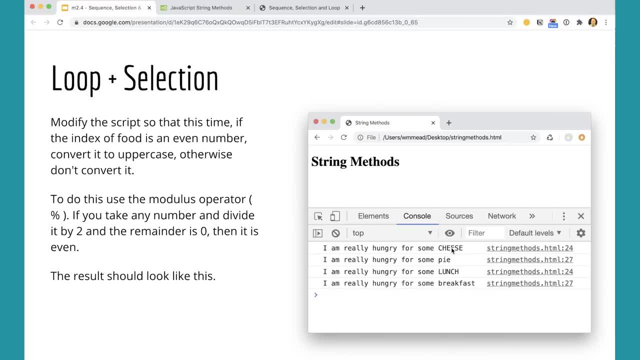 But remember, we're starting with 0.. So this is 0,, this is 1,, this is 2,, this is 3.. So these two really are the even ones. In JavaScript, you can determine if something is even or odd by using the modulus operator. 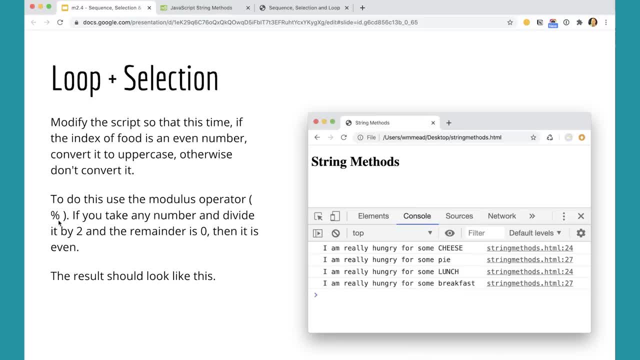 which is the percent sign. And we can figure out, when we divide something and use the percent sign, if that's even or odd. If the remainder is 0,, then it's even if you divide something by 2. So we can use that to help us figure out which of these is even or odd. 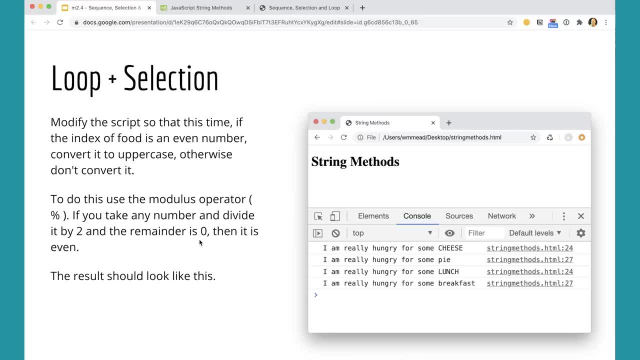 See if you can figure it out. and pause the video and see if you can figure that out, See if you can try it for yourself. You might have to mess around with the modulus operator. It takes a little getting used to, but try working with it a little bit and see if you. 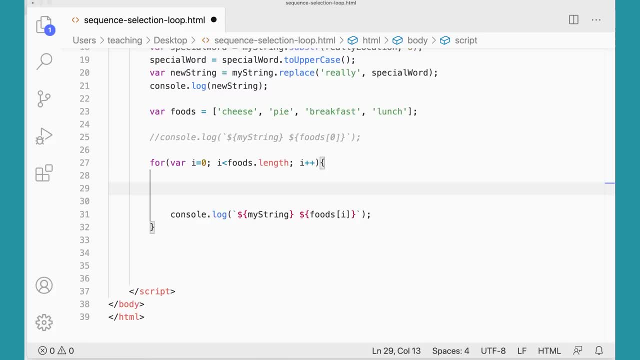 can figure that out and get this result. Let's do this together. So here I am with my loop, and I got rid of the for of loop. This one's really going to work better because we already have i working as an incrementer. 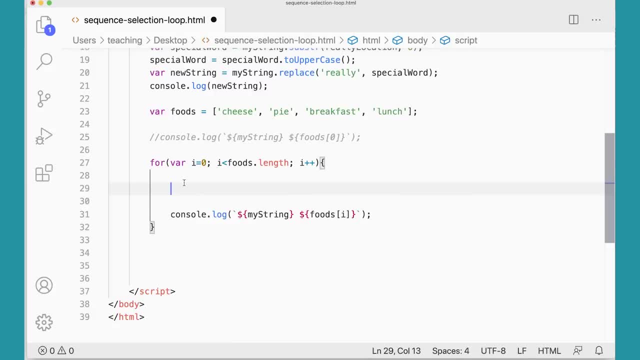 with numbers So we can just work with i to do this. So initially I'm going to add this: var remainder i percent 2.. Now what that's going to do is, each time through the loop it's going to take i and divide. 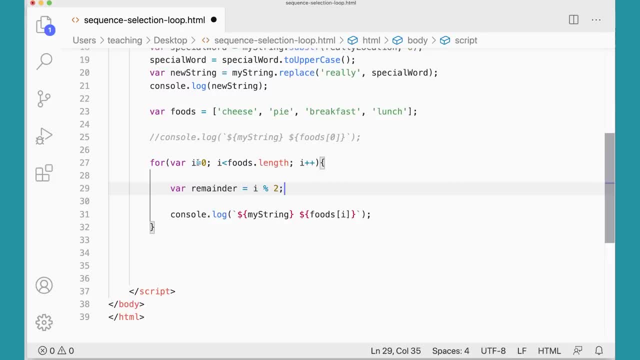 it by 2.. Let's see what the remainder is. So the first time through the loop I take 0, 0 divided by 2 is 0. So that's going to be a 0, so that's even. 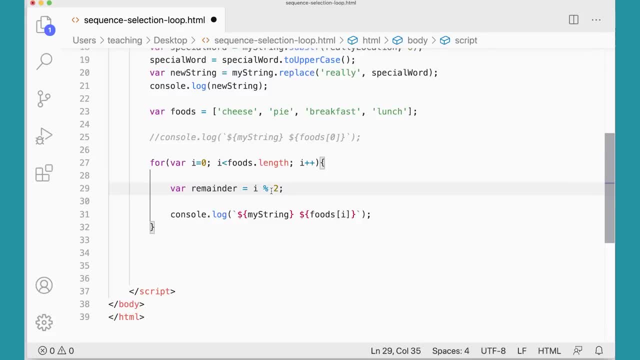 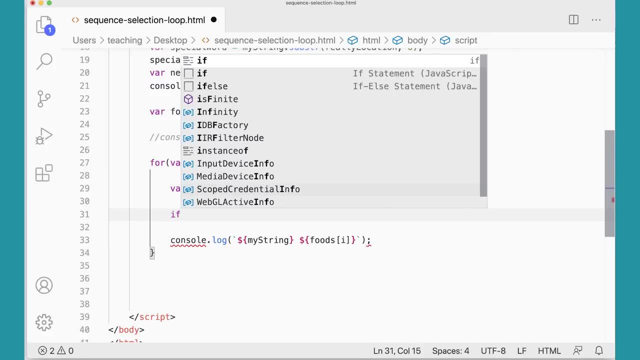 1 divided by 2 is not 0,. 2 divided by 2 is 0, so on and so forth. So if remainder is exactly the same as 0.. We could do same as, but, just to be absolutely sure, exactly the same as 0. 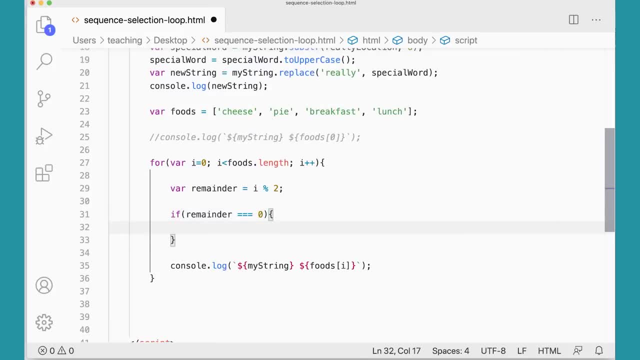 If it's exactly the same as 0, then what we're going to do is we're going to take, we're going to make a variable var food upper and assign it foods 0. 0.. 0. 0.. 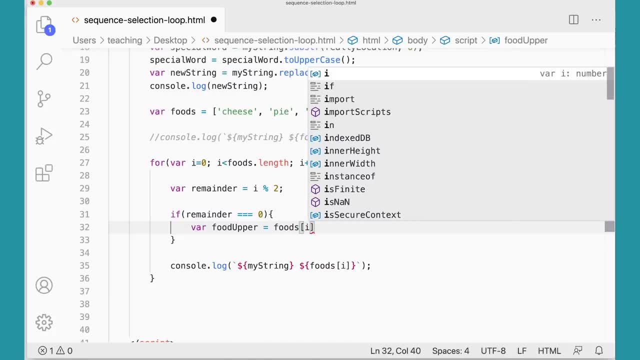 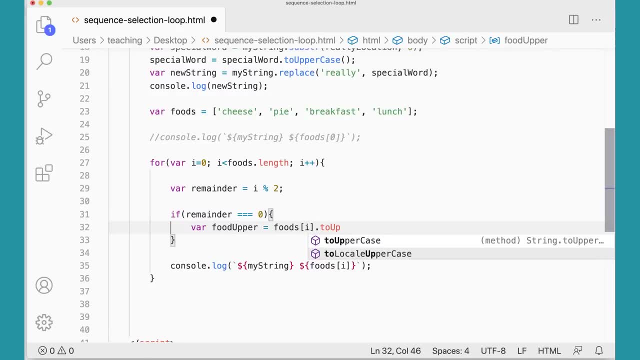 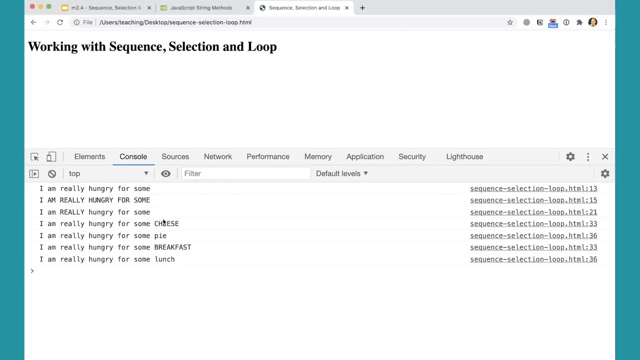 And do 2 uppercase And then I'm going to print out basically this, But instead of foods i down there I can print out this one here. I think that'll work, else we'll just do this. save that, did I do it right? let's see, refresh my page here and look at that. 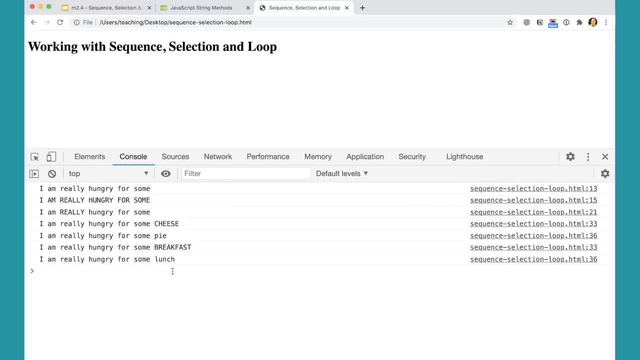 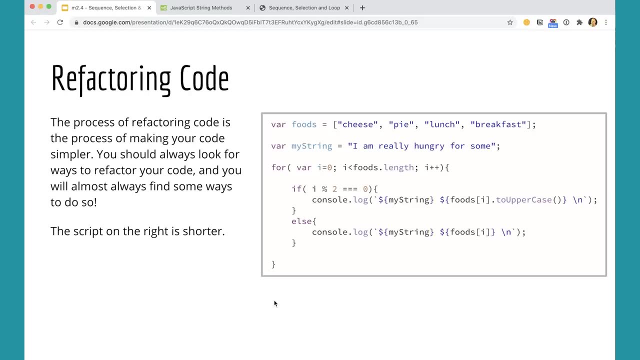 it's working, so that's great. did you get something like that? that's great. one last thing I want to talk about- or really the next thing I want to talk about- is refactoring code. often we will write code the first time and then look at it later and realize you know what. that could be a little bit simpler. I 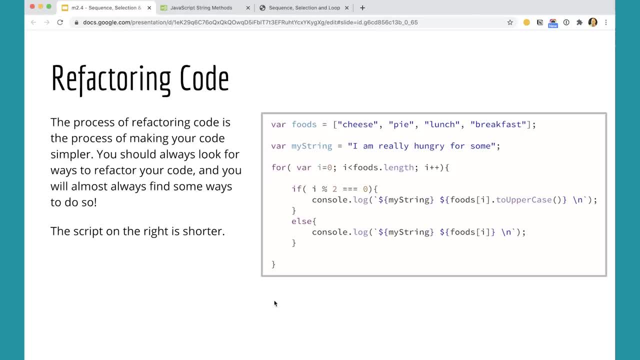 don't know if you've ever done that before, but if you've ever done that before, I need to. I could make it. I could simplify that a little bit, and refactoring code is the process of taking your code and not changing its functionality at all, but making it simpler, finding ways of making it. 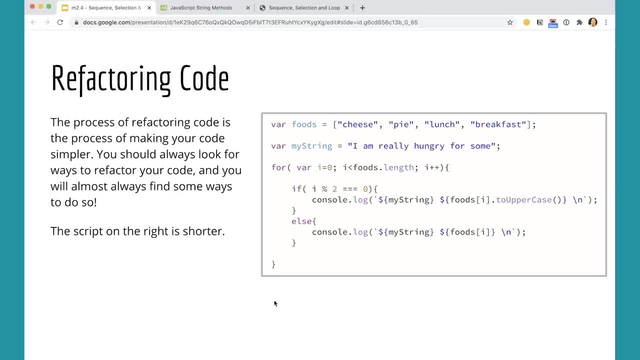 shorter, making it more concise, making it more readable. so you know, and sometimes those things don't all go together, sometimes making it more concise makes it less readable, but really you're looking for the right balance of conciseness and readability when you're refactoring your code, so we could take that same piece that we wrote. 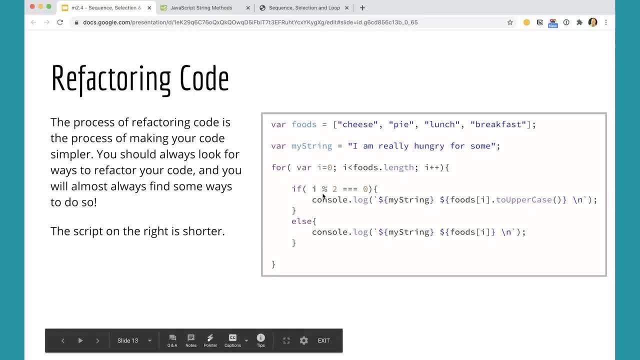 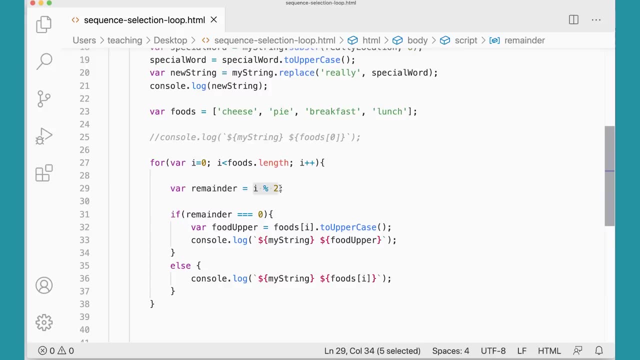 and refactor it a little bit so that we could get, so that we could get rid of that extra variable here. so let's, let's do that really quickly over here. I don't really need to do this here. I could actually do this right in here and then I 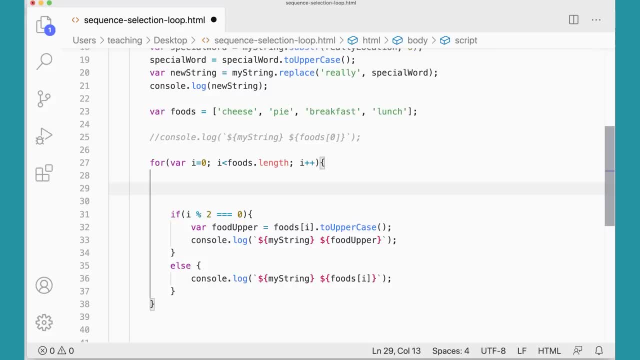 can get rid of it. so here's a nice new code. I need to add it to in here. so here's a bit more basic of code. so when I write a new code I need to add in and do it right. so here's some this variable remainder. I don't really need that there And that kind of simplifies things. 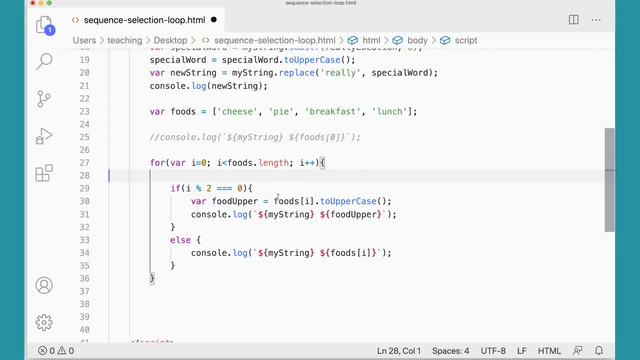 a little bit. And then here also: food upper, food upper. I could just take this foods to uppercase, food die to uppercase and stick it in here, And then I can get rid of this line too, And you can see how that sort of shortens things up a little bit Often when we're writing things. 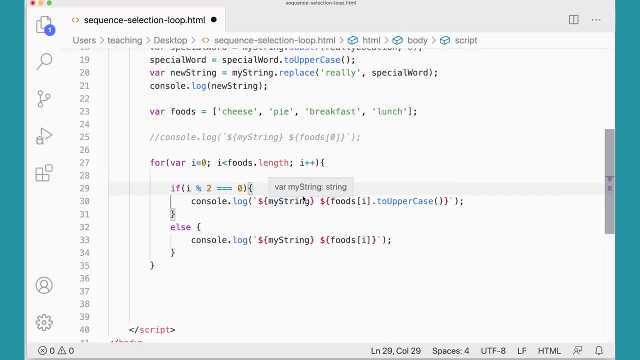 for the first time, we'll make it more complicated than it needs to be, And frequently students will tell me when they're working through my examples. they'll say: oh wow, I tried it and I ended up with way more code than you did. You know, yours was much more concise. Well, that's because I've 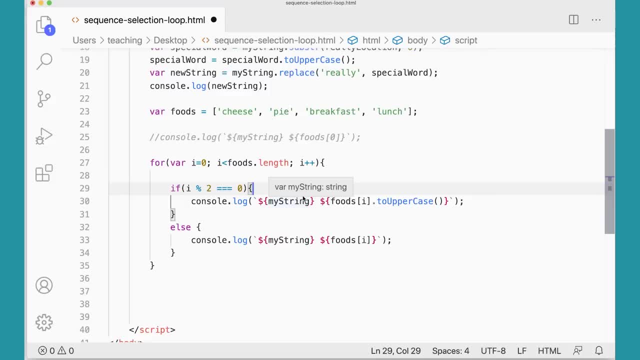 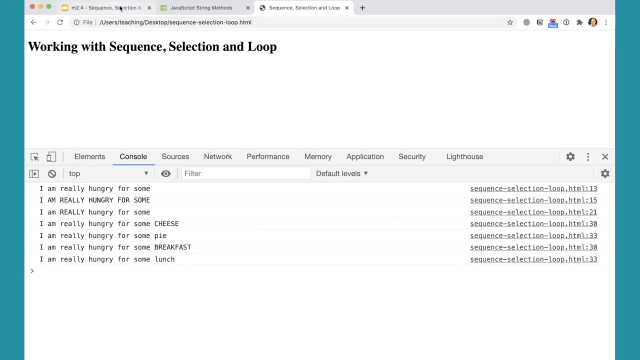 refactored mine down quite a bit. Nobody writes it perfectly the first time, So I'm going to take that, I'm going to save it and I'm going to just make sure that it still runs exactly the same way. Make sure I did that right And I did So. that's fine. Another thing you can do, that's. 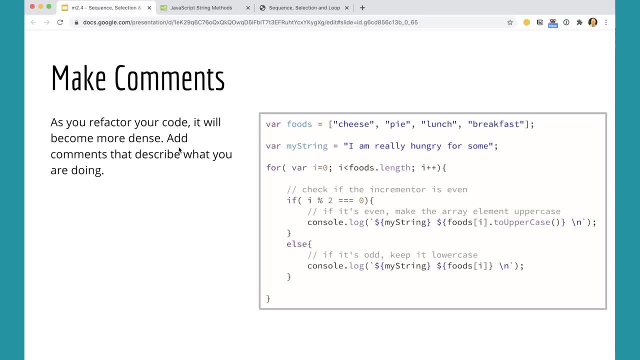 really helpful is make comments If you're not really sure that you're going to. you know you can refactor something down, but then it can become less readable and it can be helpful to put comments in there to help you make sure that you are when you come back to it later. that you know. 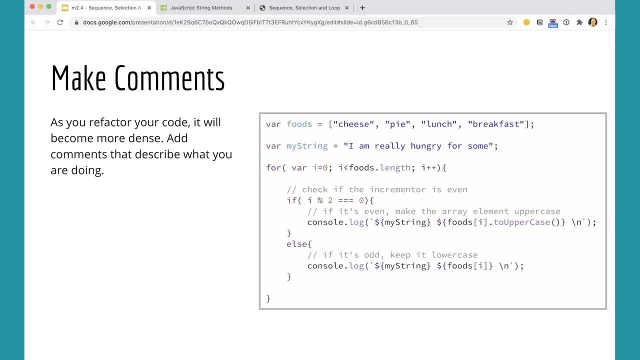 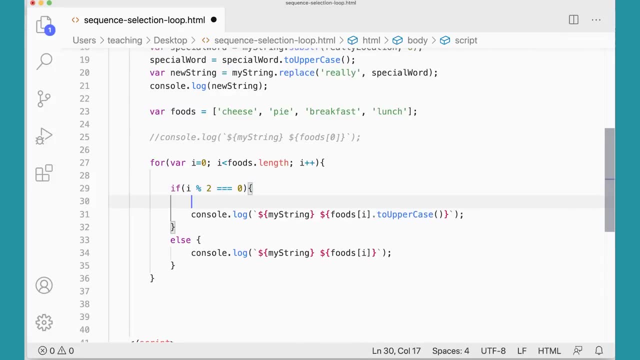 what you did and that it'll make sense to your future self. So you know you can go ahead and come in here and add comments Now I'll put it up here. Checking to see if the incrementer is even Something like that will be helpful later. 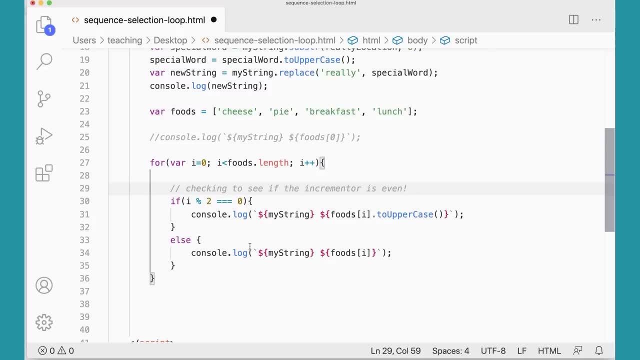 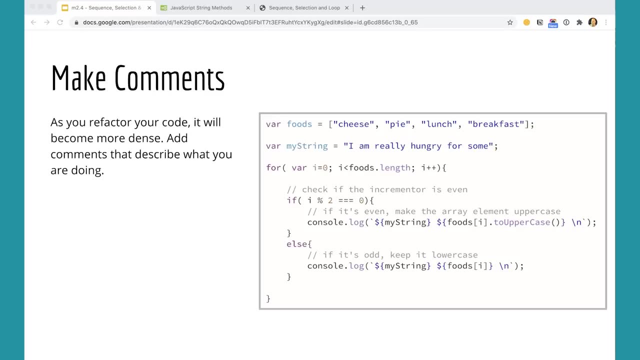 perhaps- and you could add more comments in here. So, as you're refactoring, be sure to do that as well Once you've added your comments and refactored your code. you've done a great, great job at working with sequence selection and loops And we're going to get more practice. 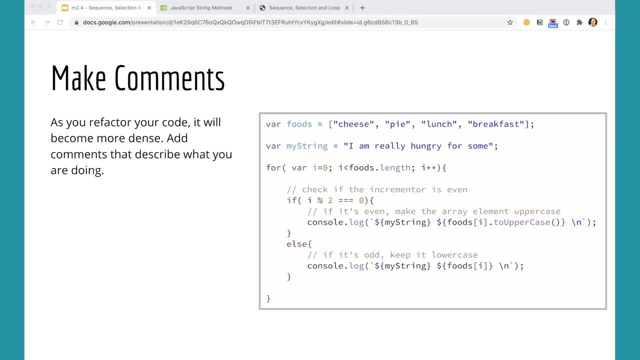 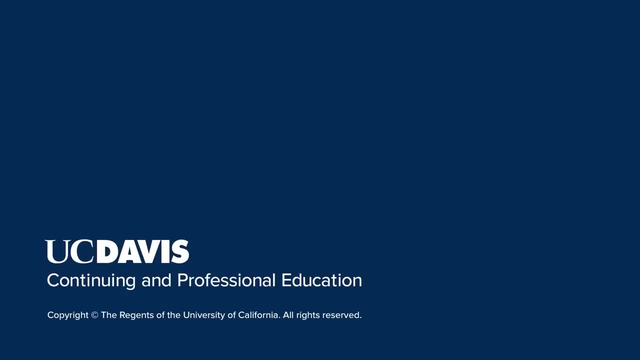 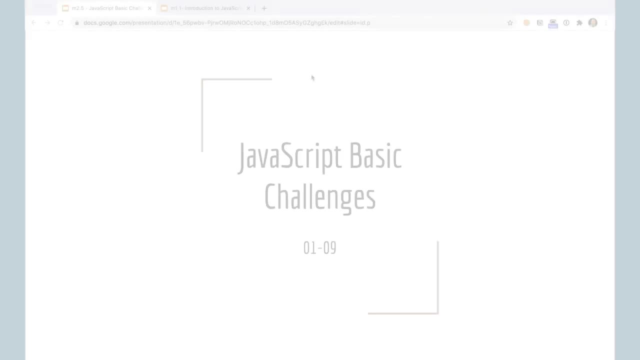 with those, as pretty much every script that we write will have some combination of them as we go along. Okay, great, See you in the next lesson. JavaScript Basic: Challenges 1 through 9.. This course includes a number of challenges, and these challenges will really help you become better at writing JavaScript. 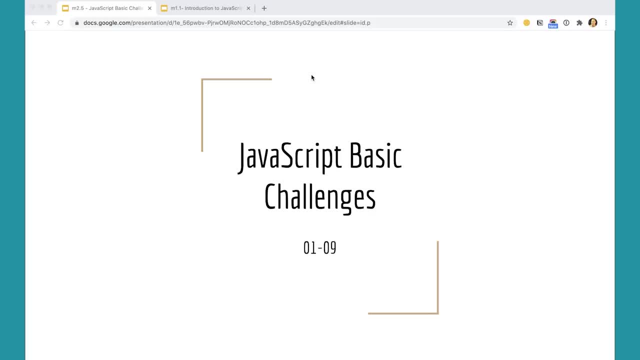 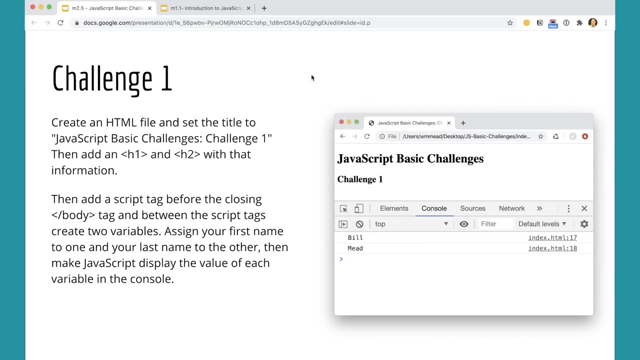 and becoming a JavaScript programmer. So I strongly encourage you to take the time you need to to get good at working through these challenges and to really be able to do the challenges and get the correct results. The way the challenges work is. I'll give you a. 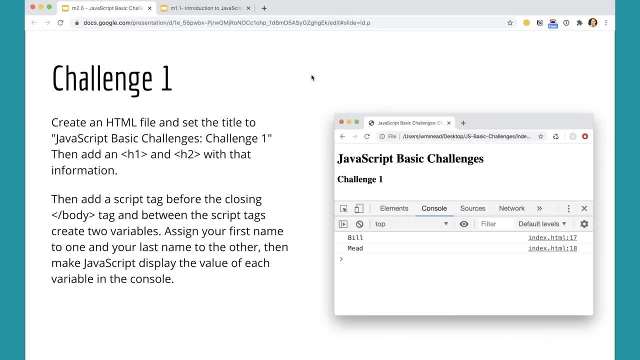 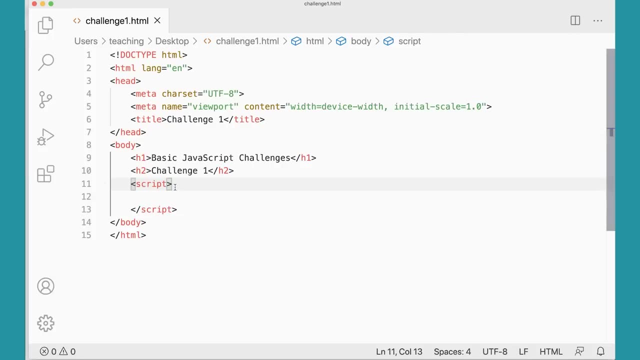 challenge? This first one is fairly simple: Write a script that prints out your name on one line- Your first name- on one line, your last name on the next line. Very basic challenge. But what you should do is set up your file. So I have a file set up here And then you'll come in here And 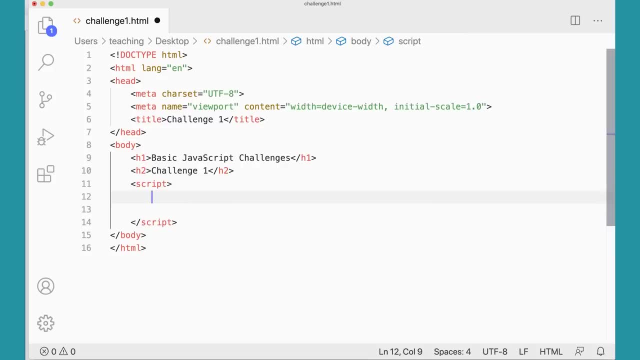 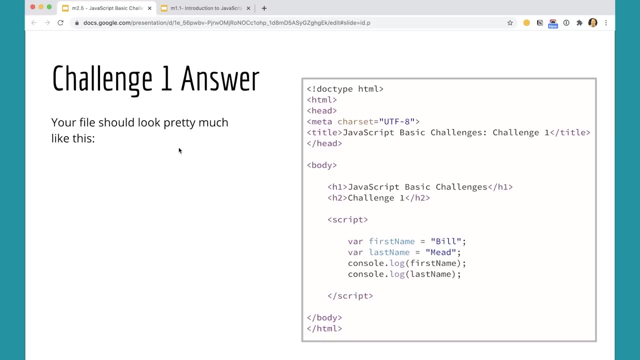 it's very normal to be: okay, what do I do first? I don't even know what the first thing is to do, And that's fine. You can always come over and look at the answer, for the challenge will be on the next slide And you can look at that and go: Oh, okay, Yeah, yeah, yeah, that makes sense We. 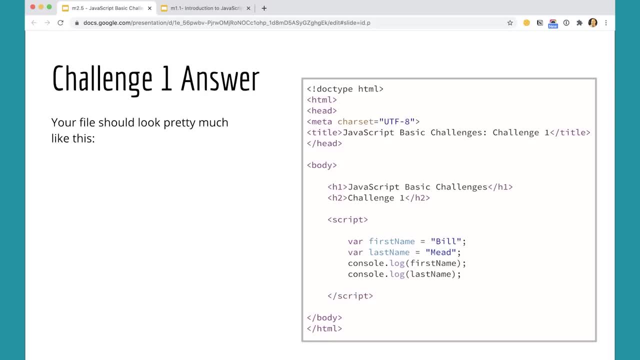 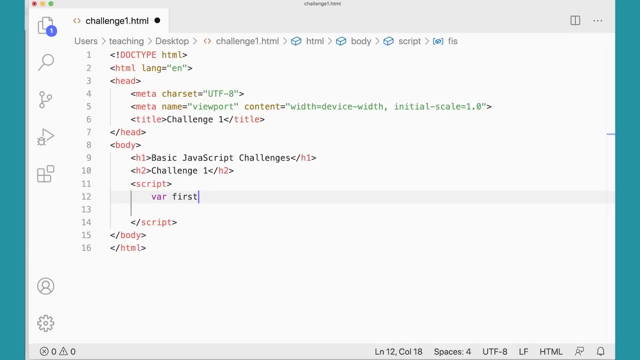 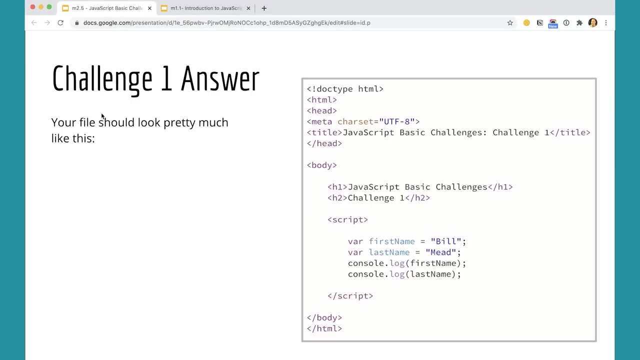 did that in in the other lesson. I know how to do that. So then come back and actually write that bar: first name equals bill. And then, oh, I've forgotten what to do next. And that's normal, This is typical. So go and look again, if you have to look again and see what you need to do next. And 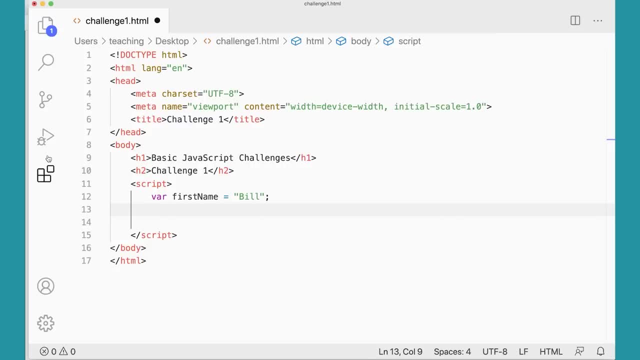 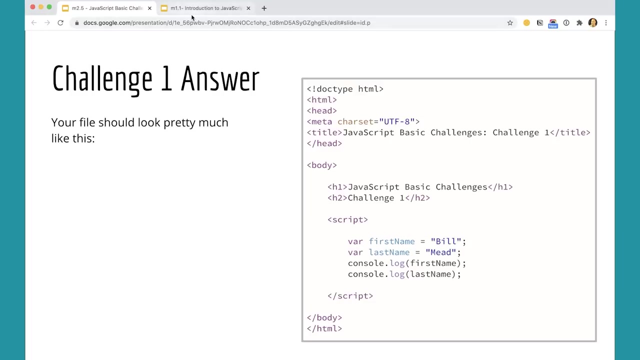 then go back and actually type it without Looking at the slide. What this will do. this will do a few things to really help you get good at JavaScript. First, what it will do is it'll help you with the syntax of the language. Remember this. 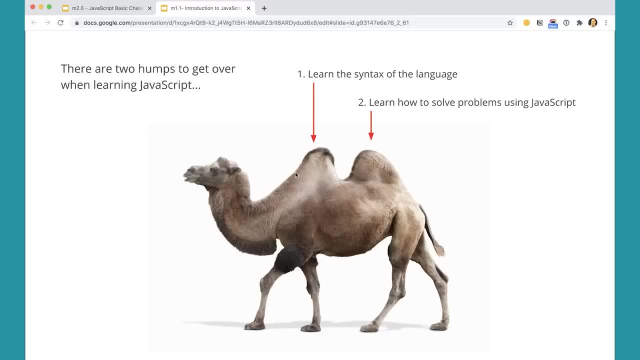 slide. Remember, we need to get over this first hump of the camel. we need to get over that first time, which is learning the syntax of the language. And the way to learn the syntax of the language is to type it And 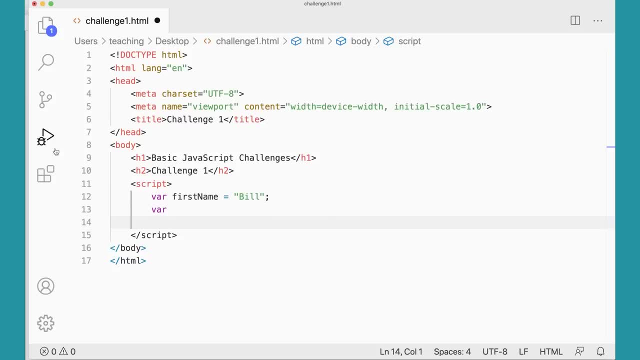 when you're working on this, even if you're looking at the answer and then having to come in here and just remember it for a few seconds. that will help you learn the syntax and get better at it over time, And I promise it will help. Over time you'll really start to be able to do these without having to. 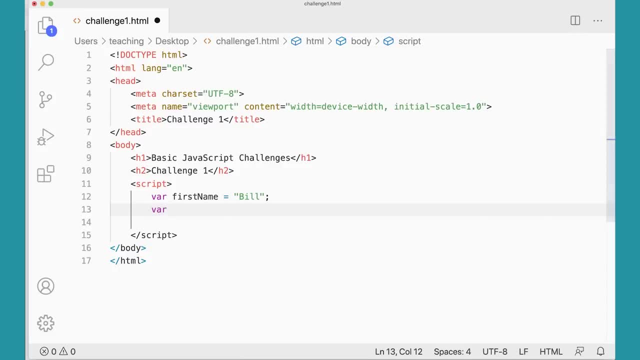 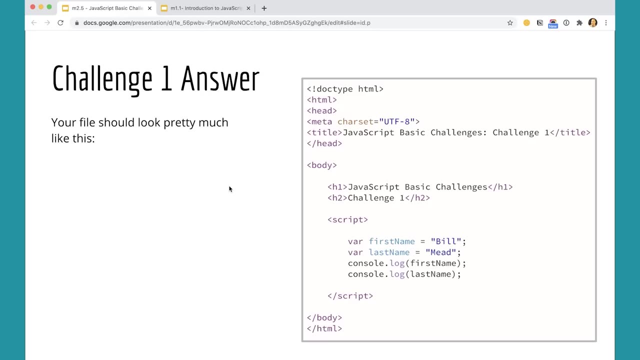 look at the slides if you keep working at it. So look at the answers if you have to. they're here And then type it without looking at the answer. The second thing that it'll do for you is these challenges build on each other. 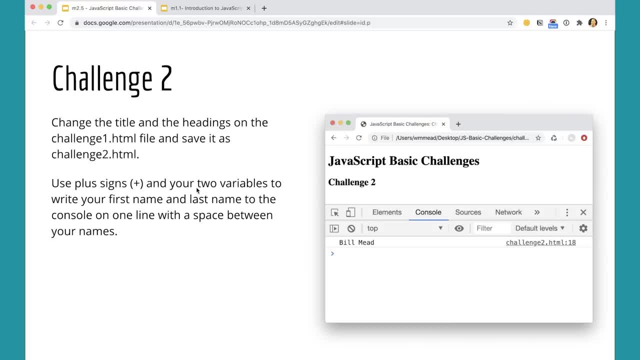 So the second challenge is a little bit of a baby step beyond the first challenge, And I've designed these challenges such that they build up in small baby steps like this, so that over time you're taking an idea and kind of expanding it, expanding it, expanding it into a larger, more complex script. 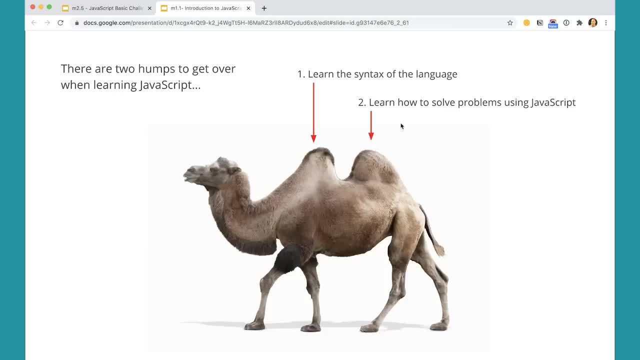 as you go along And that will help you With the second hump on the camel, learning how to solve problems with JavaScript. You get learn good at learning how to solve problems first by solving very small problems and making baby steps, And that and these challenges will help you do that. So I recommend you do these challenges. 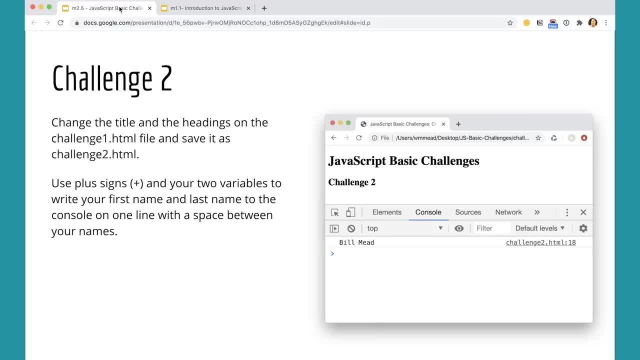 to the point where you can do them without looking at the answers, because that will really help you with the syntax And meanwhile you're building up some skill for how to take a small thing and then build on it. Now, there's nothing magical about these challenges. I also recommend 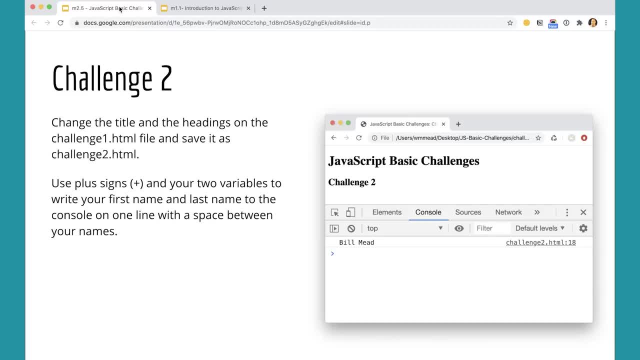 you come up with your own challenges. Try things out, See if you can make a small thing work. If you can make that small thing work, then build on it and see what other ideas you have and see if you can build on those. That is a great way to learn JavaScript And it's fun. It's fun to see if you 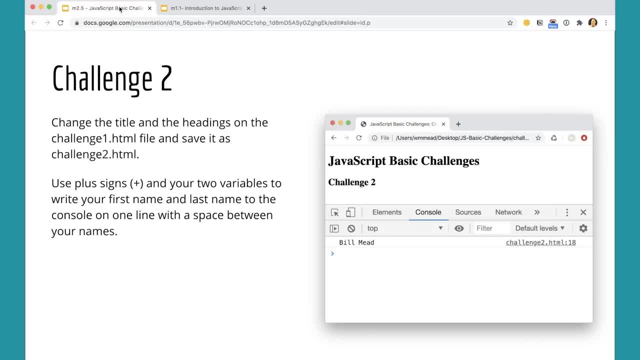 can do that kind of thing. So by doing these challenges, by working through these examples and by getting really good at them, you will build your skills with JavaScript. If you don't, you don't have to. You can continue to watch the videos and do the quizzes and the videos and you'll learn about. 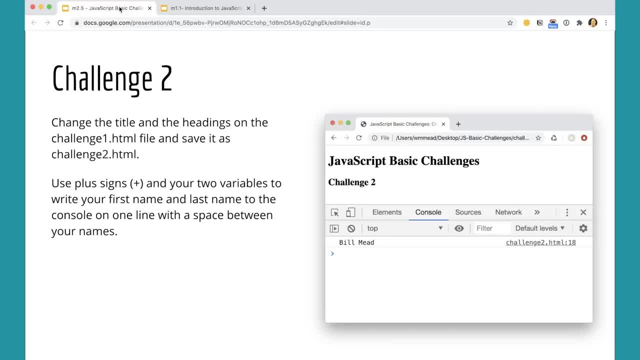 JavaScript. But in order to actually become a JavaScript programmer, you have to write JavaScript. You have to take the time to really sit down and write it, Even if you're coming to JavaScript from another language, like C++ or Java or Python or some other language. 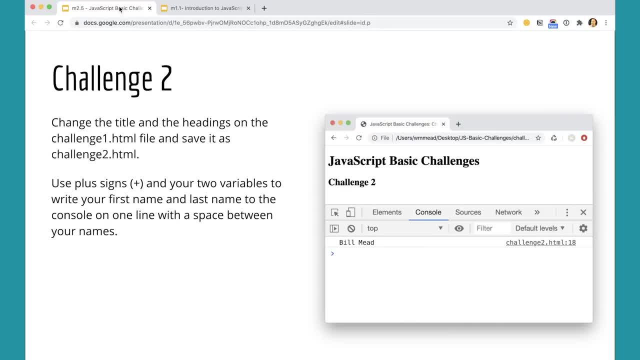 and you might be thinking: Oh yeah, yeah, I know what loops are and I know what the loops are And and I know what the statements are and those kinds of things. I really recommend you sit down and write JavaScript, because it's a little bit different and it takes practice. 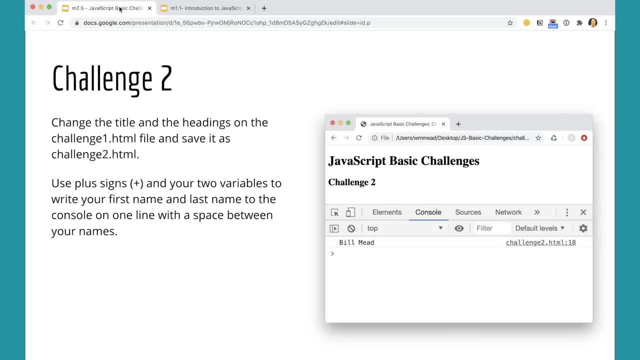 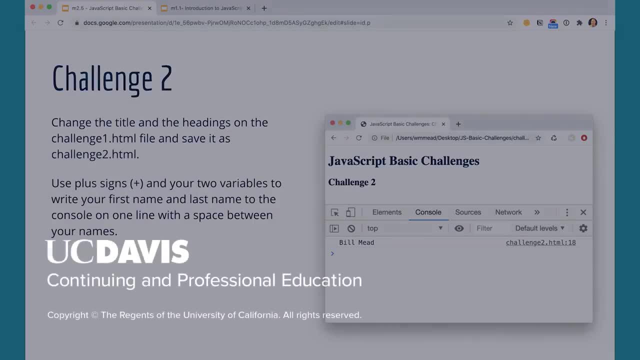 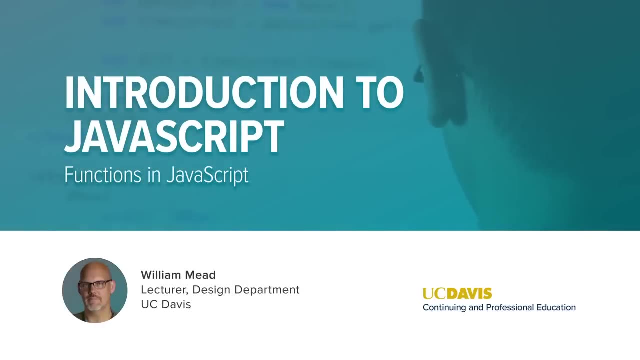 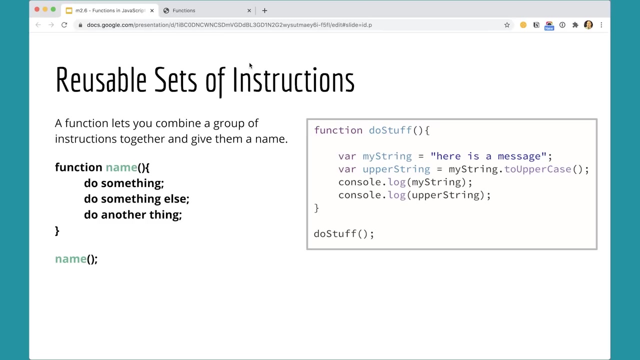 Okay, great. So keep working on these and get really good at the challenges, and you will be- I promise you'll be- on the road to becoming a good JavaScript developer. Functions in JavaScript Functions are reusable sets of instructions. So, for example, in the sequence selection and loop exercise. 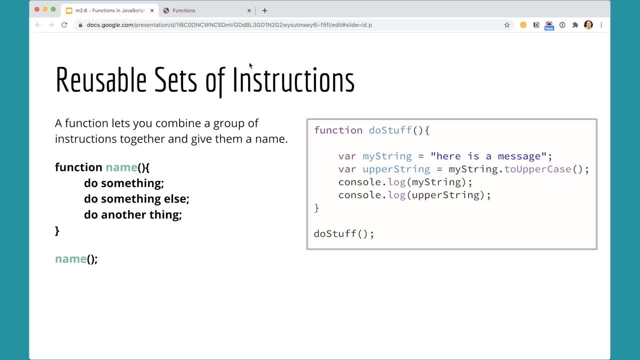 you were adding a bunch of scripts to the page and it was getting kind of messy. There was a lot of single lines of code all kind of piling up without a lot of order or organization to them. What we can do with functions is we can take that stuff. 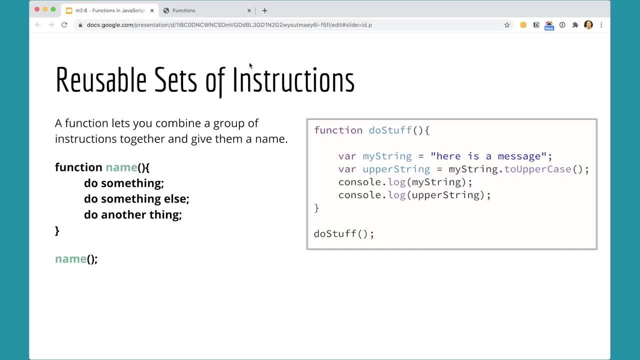 stick it inside of something that has a name and then run that function when we want to run that set of instructions. We can make functions so that they're reusable, so that you can use them in multiple places within your programs, And that's where functions can become very powerful. 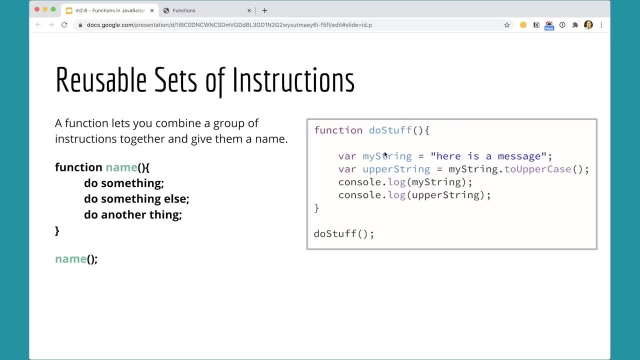 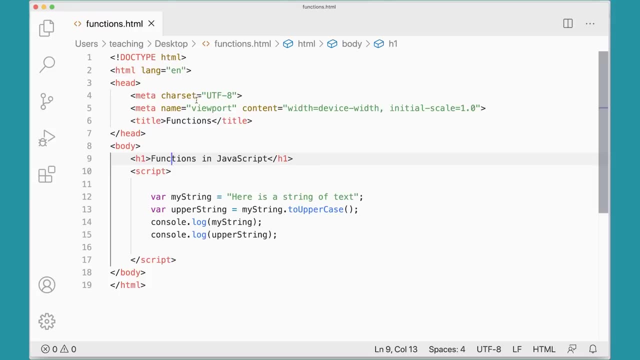 So here I have a function called doStuff which is going to run something similar to what we did in the sequence selection and loop exercise. So let's give this a try real quick. I'm going to switch over to my code editor And you can see I've already set up a file. 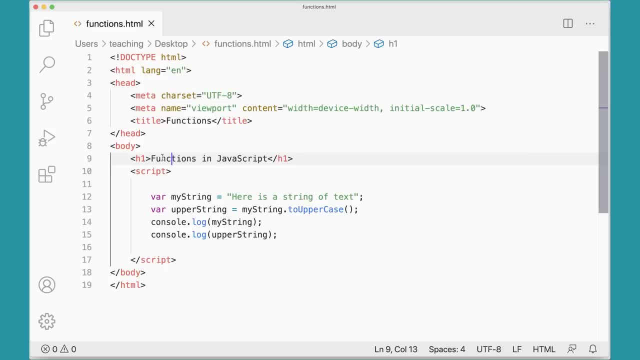 and I recommend you do the same. It's just an HTML file with an H1, and I've got a script here And I've got some of the script from our sequence selection and loop exercise, And now I'm going to add a function. 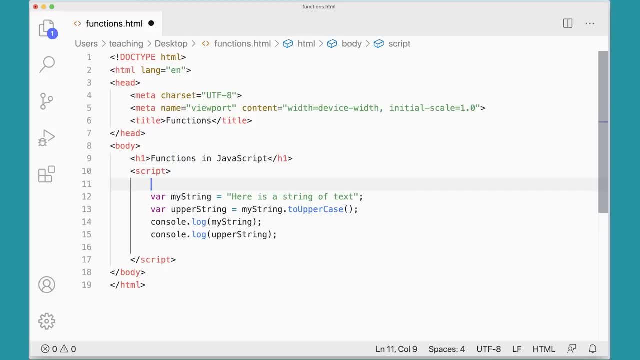 So to do that, I would just define a function here. Function: Use the function keyword DoStuff. Parentheses and curly braces. Now, this stuff can just go inside the curly braces. Like that It's probably best to tab it in. so it's clear that it's all inside there. 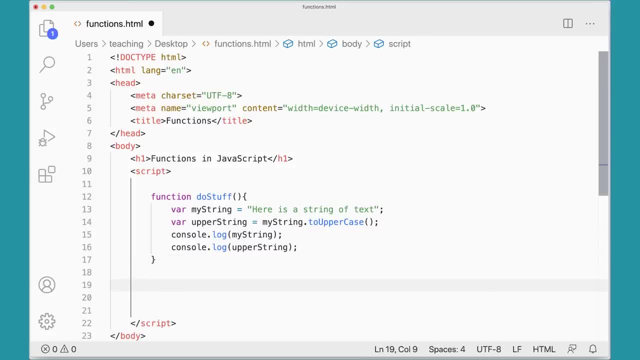 So that's inside of there. And then you have to run the function DoStuff. So we define the function which tells it what it does. Then we invoke or call or run the function. Any of those verbs will do: Invoke, call or run. 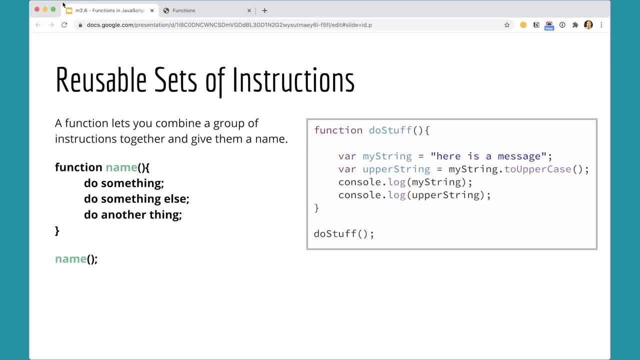 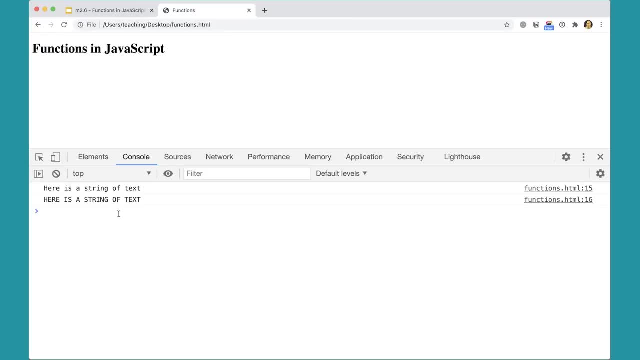 So I can save that and I can come over to my page here. So this is that same page And I can run this and you can see that the function runs And it does its thing. It's very nice. It's very normal when you start doing this, and sometimes I still do it. 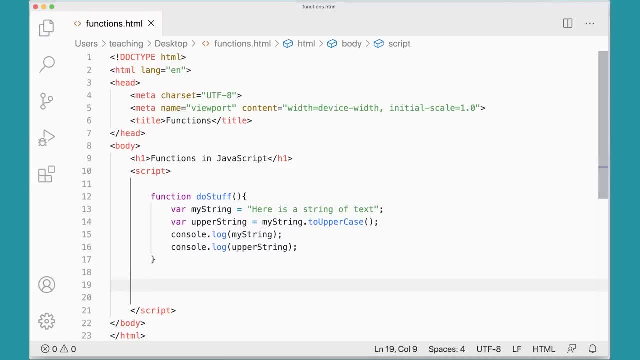 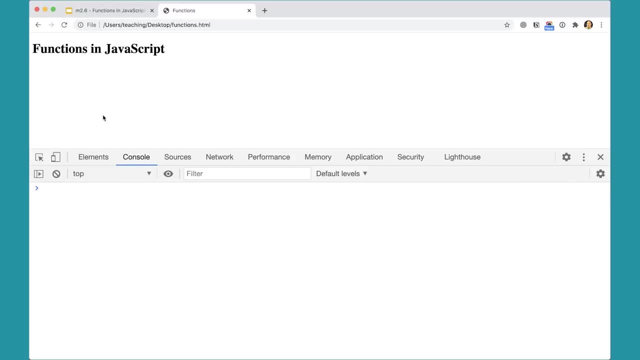 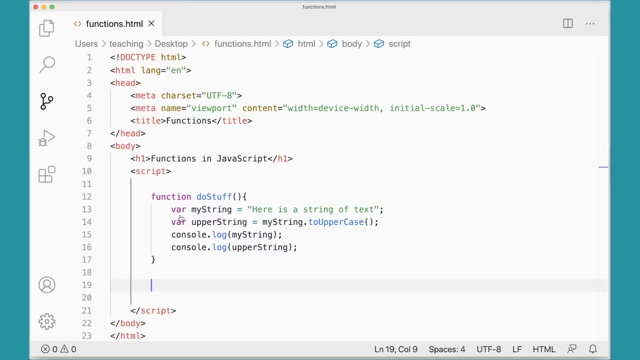 to forget to call the function, which will mean that you'll get nothing, Because it will be defined but it won't actually run. So it's not actually running there. I have to run DoStuff, Okay, Okay. So normally I would do that here in the file. 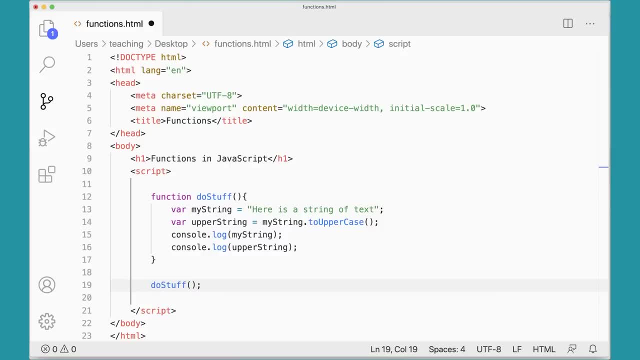 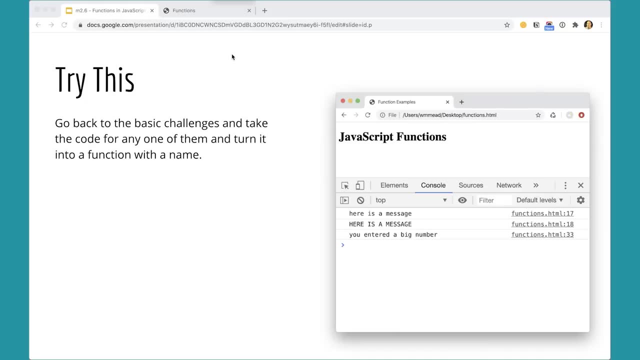 DoStuff, We'll run that function. Here's a good thing to try. Go back to the basic challenges that we just did and pull one of them out of there and turn it into a function. I used challenge number seven, but you could use any of them really. 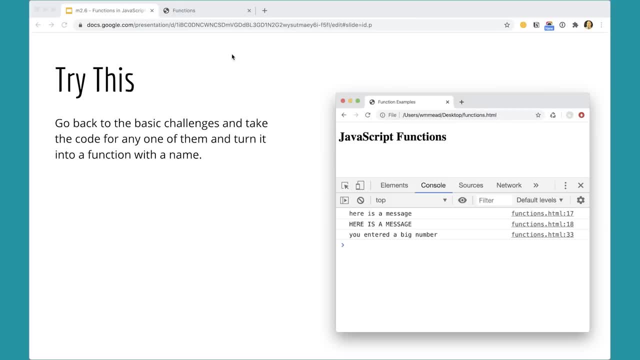 See if you can turn it into a function and run it and pause the video, and when you come back we'll see what you got. I hope you were able to try that. I went and got a challenge. I went and got challenge number seven and I have it over here. 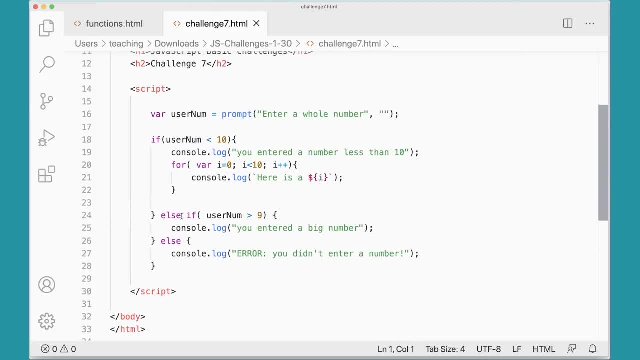 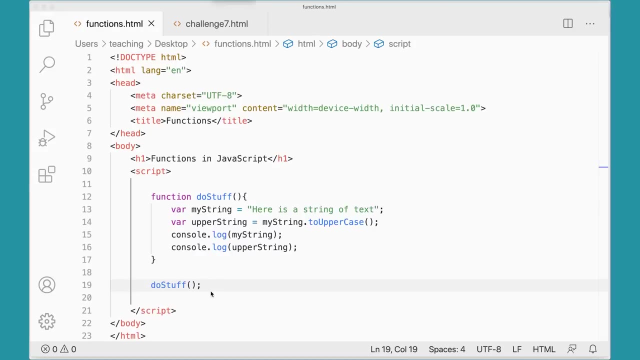 So here's challenge number seven: How would I take that and turn it into a function? Well, I could do it like this: I could take all of this stuff and I could come over here and I can go ahead and just. 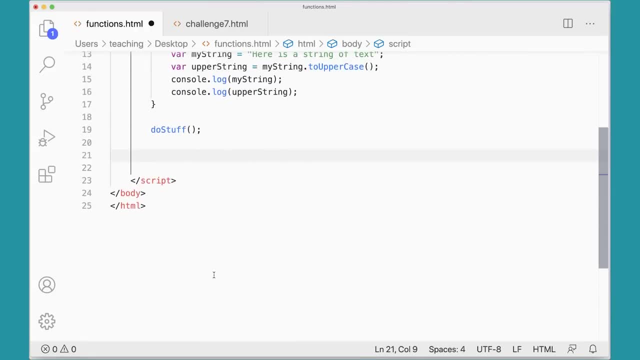 paste it right on my page here, right in my file, here down here at the bottom. I'm going to just paste it on in there, But I'm going to make a new function And you know what is this thing doing? 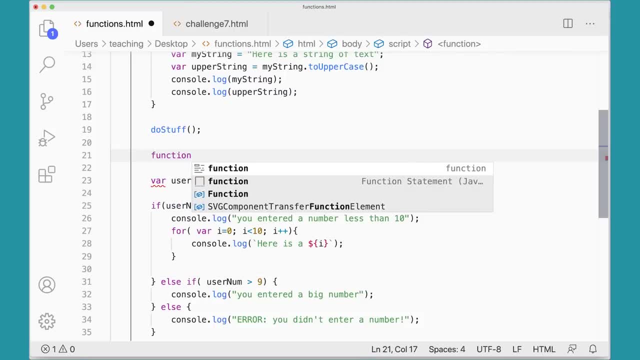 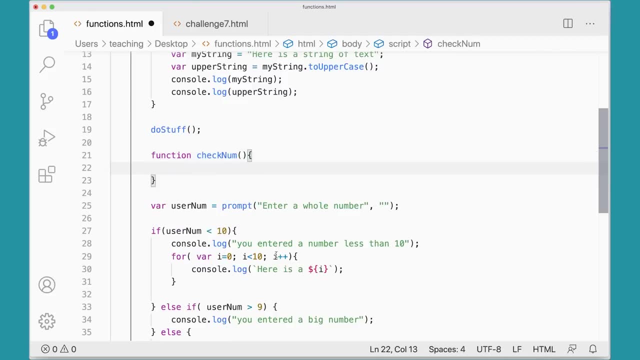 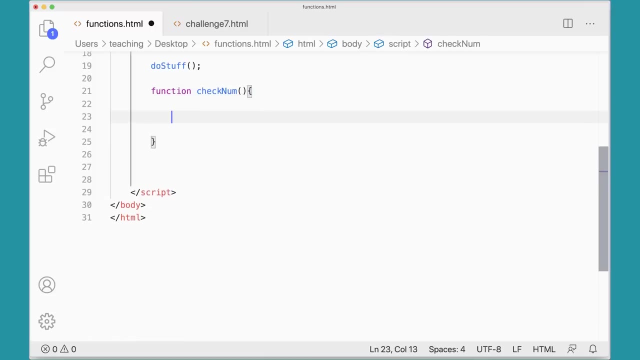 Well, it's checking a number, So I'm going to make a function called checkNum- parentheses, curly braces, like so- And then I'm going to take this stuff and I'm going to stick it inside of checkNum. I'm going to tab that in, so it's clear that this curly brace 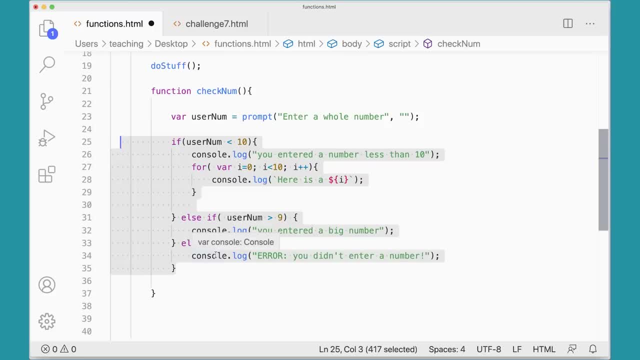 is ending that curly brace and that everything is inside. It's always good to be clear about your indenting. if you possibly can, It really does help. And then down here I'm going to run checkNum. Let's see what happens. 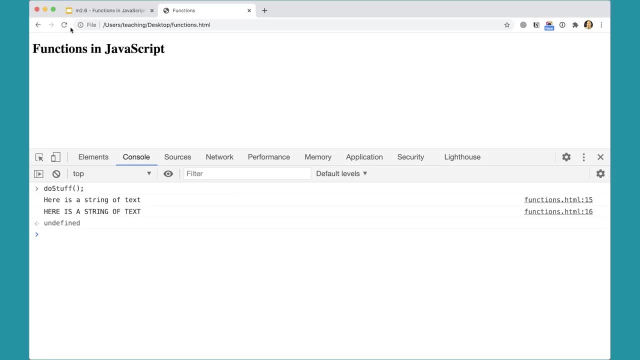 So over here, when I run my script, it says: enter a whole number, 54. And then you entered a really big number. So my function is running, it's functioning, it's doing what it's supposed to do And all that code is now inside of a function. 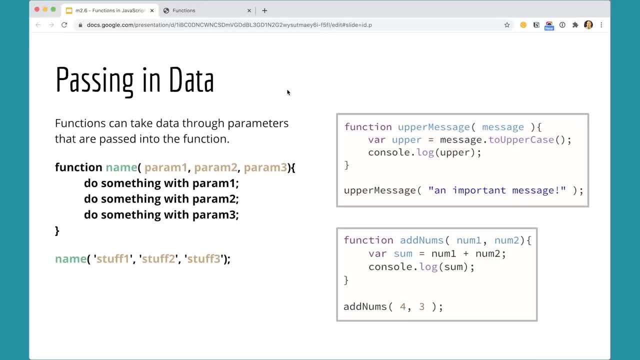 Functions are even more useful if you can pass data into them so that they can do something with that data. So, for example, our first doSomething message, the first doSomething function, wasn't really useful because it was just taking that string and making it uppercase. 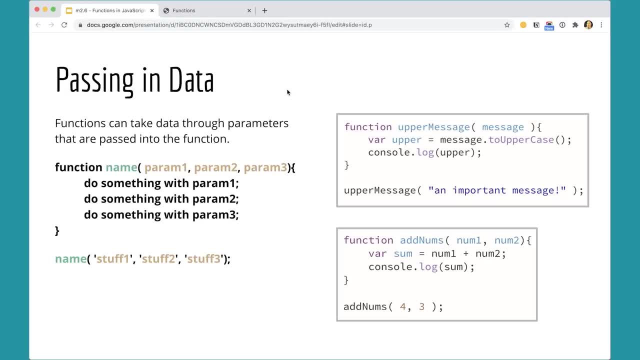 and spitting it back out again. But we could make it more useful by passing in a message variable, a parameter. This function has a parameter called message. We could pass in and messages, an argument to this function and it'll take any message and make it uppercase. 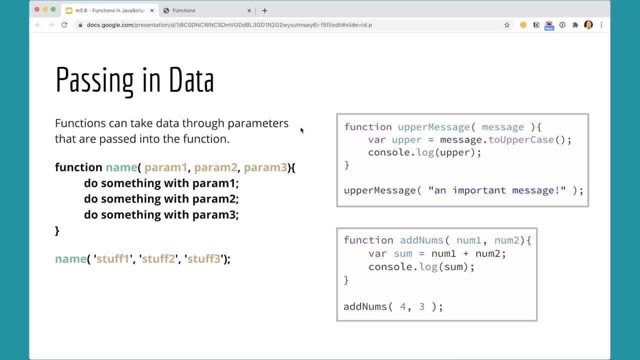 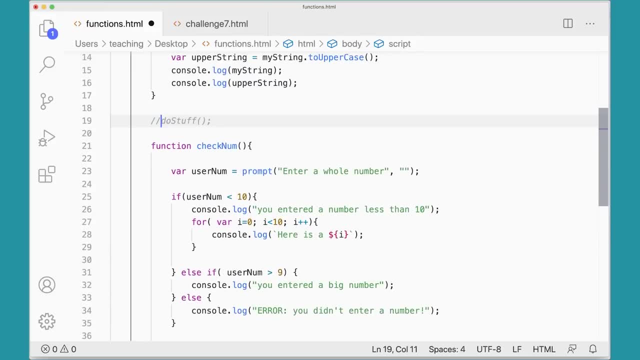 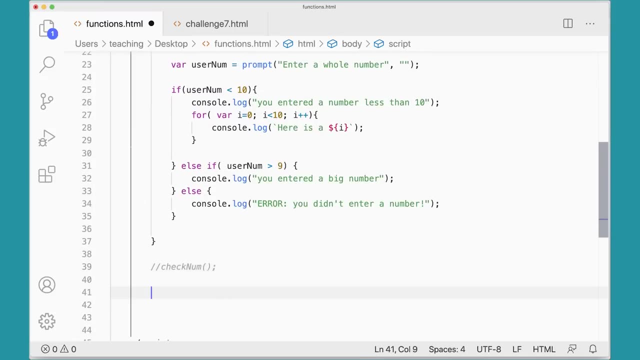 and console log it out. So let's give that a try and see what that does Down here. I'm going to comment these out. I'll leave the functions. they're not going to hurt anything. I'm going to comment these out so they don't run, And then I'm going to make a function. 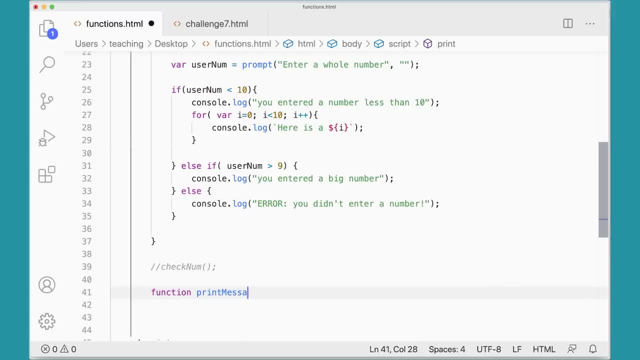 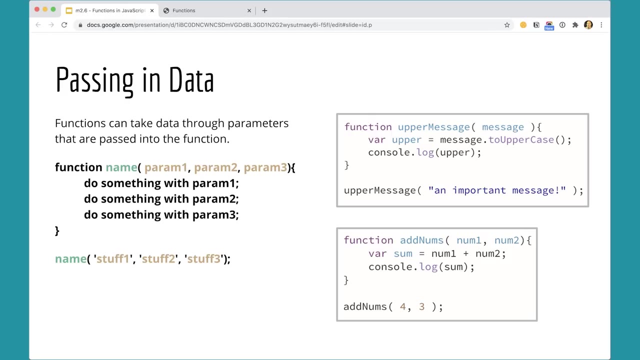 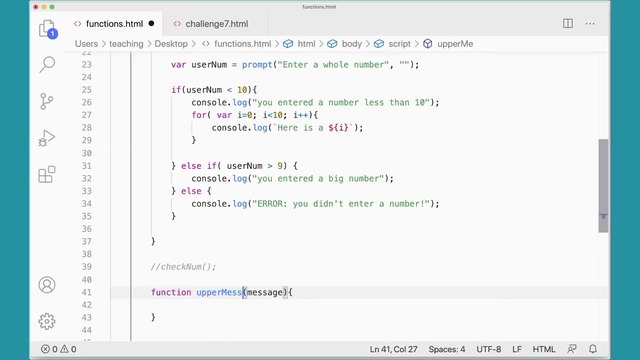 function. print message, which takes message as a parameter, or print uppercase, or I forget what did I call it over here? Probably shouldn't make it match with them. Print upper message. Let's do that then. Upper message. It doesn't matter really what you call it. And then I'm 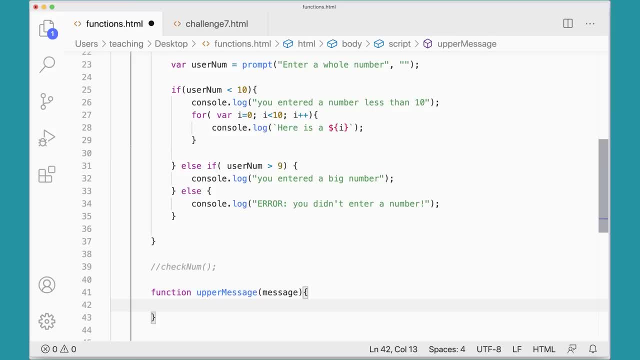 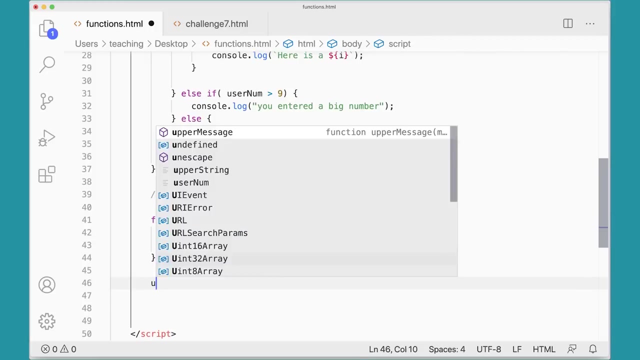 going to take message And I'm going to say: you know, var upper message equals messageto uppercase, And then I'm just going to console log out upper message. Now when I run this I run upper message that I pass in. Here is a message I can pass any message in that I want. 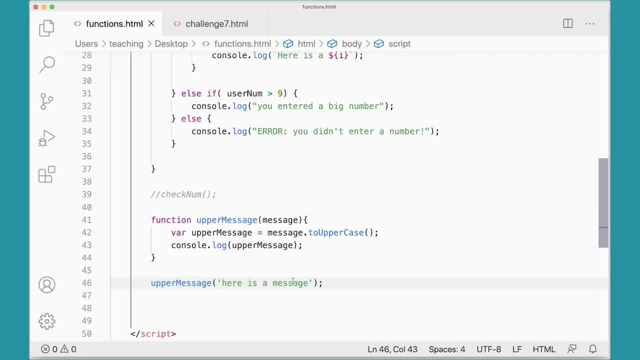 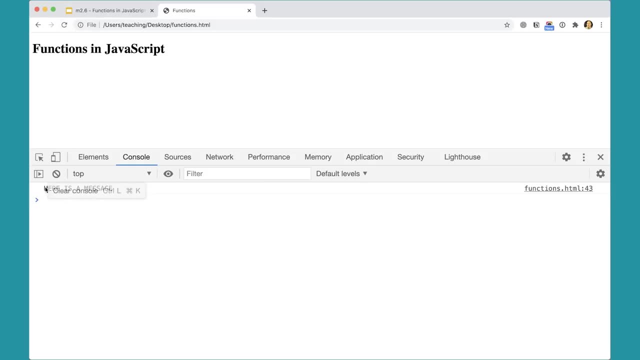 and it will make it uppercase- Still not super interesting, but you know, it's something that shows us how this actually works. So every year when I run this, my message is turned into uppercase, because that's what that function does. It takes some data and does something to it. 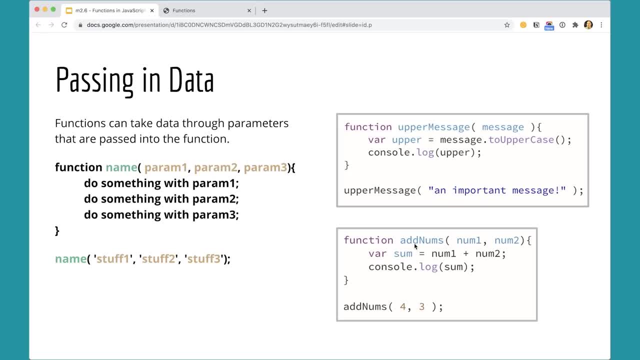 And beyond that we could do something like add numbers together- Again, not super exciting, but we could pass in two parameters here, a number one and a number two. We could add them together and then console log them out, And you would run this by using add nums and you would 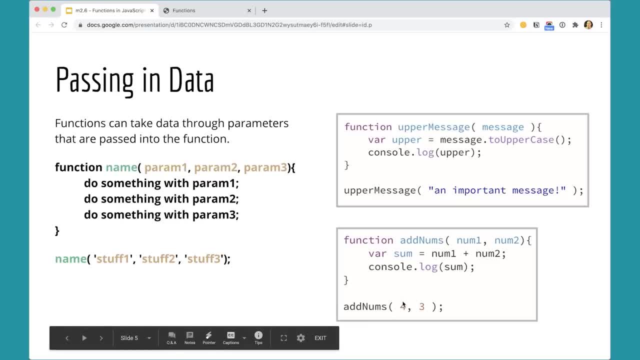 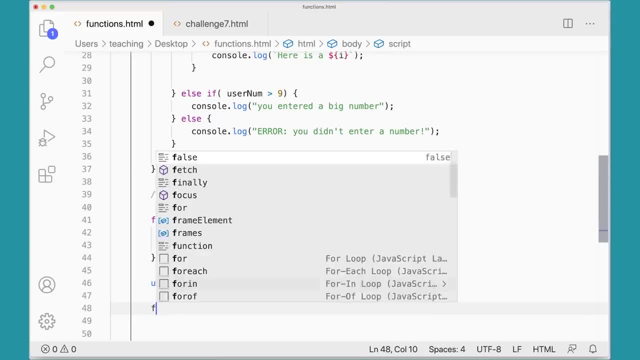 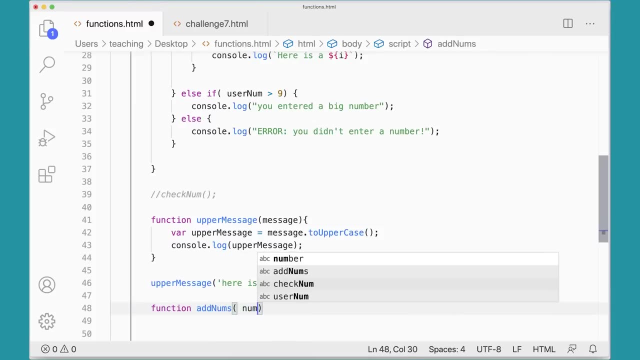 pass in whatever two numbers you want to add there. Let's give it a try real quick. So function add: Add nums. We're going to pass in num one and num two. I like putting these extra spaces in here, even though that's kind of not the standard, but I think it makes it easier to read for me. 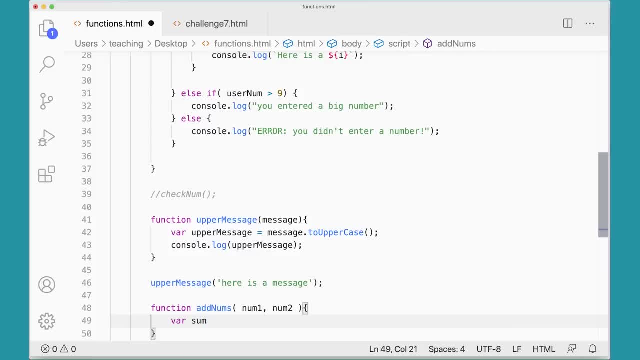 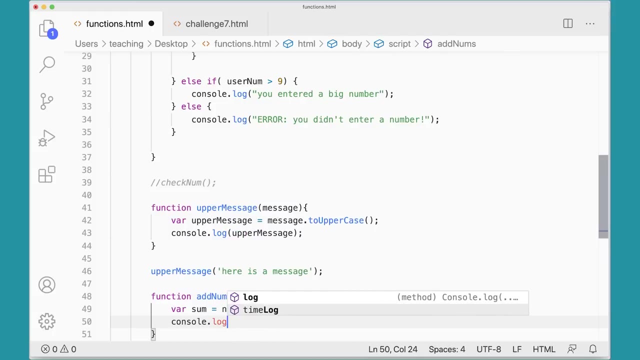 All right. So I'm going to make bar sum equal num one plus num two, And here we're using the plus sign to actually do addition. That's what we want it to do. And then I'm going to console dot log sum. 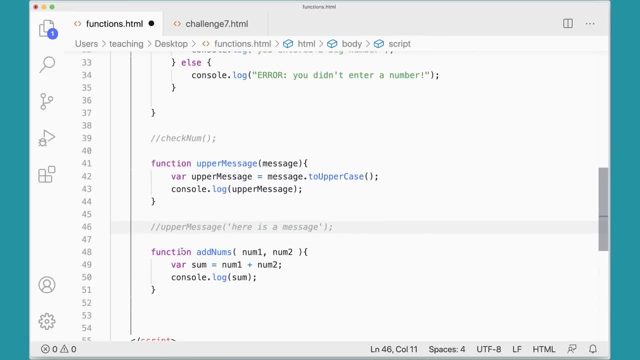 Meanwhile I'm going to comment that out so we don't get that running as well. And then down here I just need to run it with whatever numbers I want to add: Add nums 329 comma 490.. And then I'm going to run it with whatever numbers I want to add: Add nums 329 comma 490.. 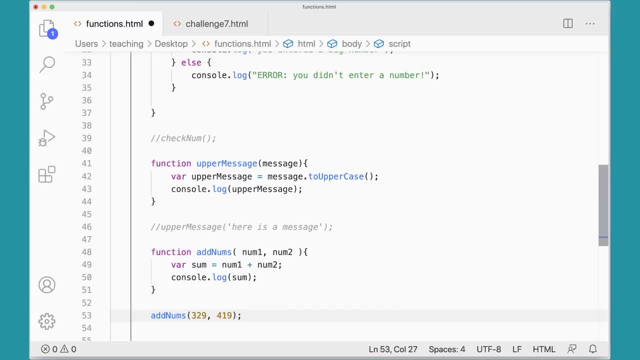 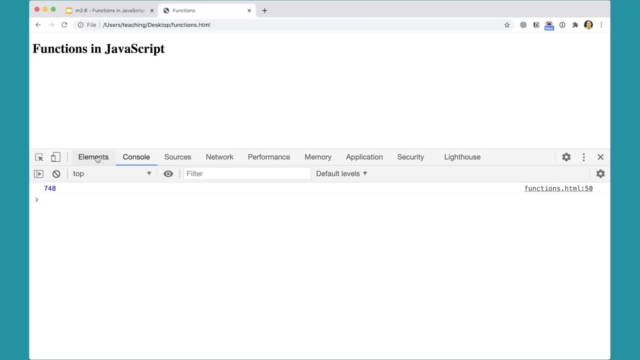 Sure, you could probably do that in your head fairly quickly, but you know why bother. We can have JavaScript do it for us, right? So if we're going to learn how to do this JavaScript stuff, we might as well do something useful like add those numbers together to get 728. 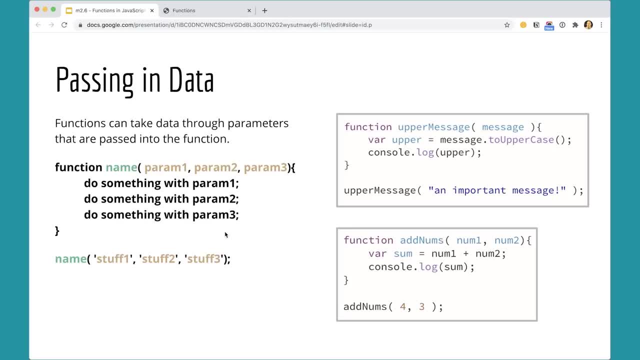 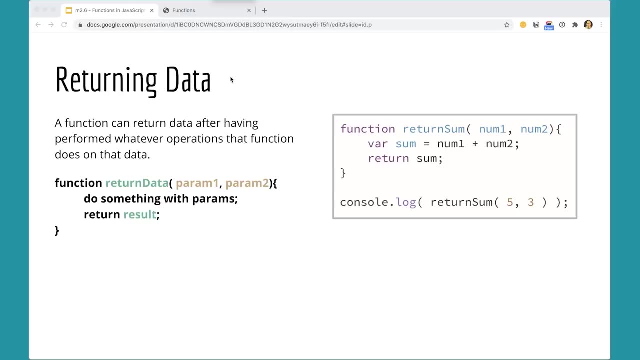 Maybe not super useful, but you get the idea, And that's a really powerful thing about JavaScript is we can pass in the pass in data through these variables here That we can then work with within our function. The next thing to talk about is returning data. 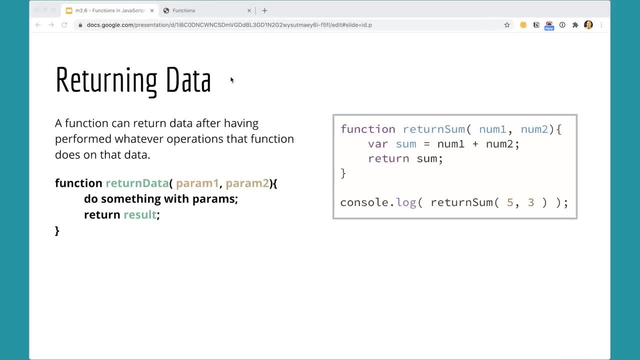 So far, our functions have just done one thing: They've printed out to the console log. Because that's really all we have for right now. We will be doing more interesting things, I promise, But for right now what we have is to print out to the console log. 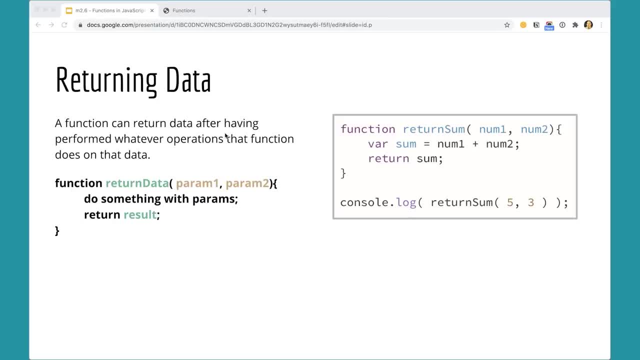 But we can make functions that return something And that in this case it looks subtle. The difference is subtle because in the end what we have is the console, so we're printing to the console. But here I've updated my function. I'm calling it returnSum. 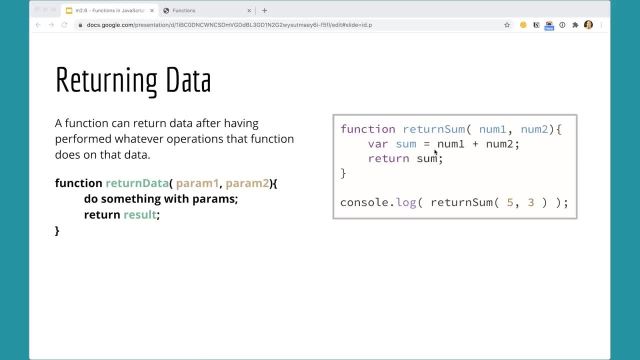 And instead of just printing to the console, I'm returning the sum of these two numbers And then I can console log that out Again. it's just going to the console, so the end result isn't all that different. But there is a subtle but important difference between these two things. 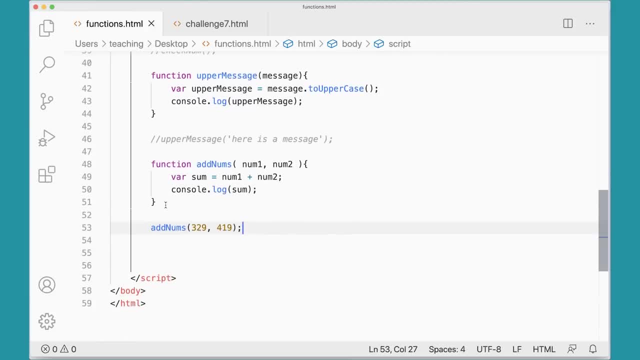 Let's do this really quickly. I'm going to come over here and I'm going to just copy my addNums function and paste it. Comment that out for a moment And instead call this: returnSum num1, num2.. But instead of console logging it out, I'm going to return return as a keyword sum. 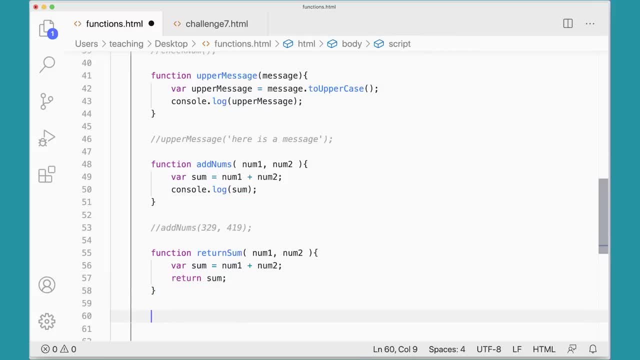 So it's going to return the value here And then I can again. it's just going to go to the console log, because that's all I've got access to at the moment. We'll be doing more stuff later And I can run inside the console log- return sum- and I can put a 3 and a 5 in there, whatever. 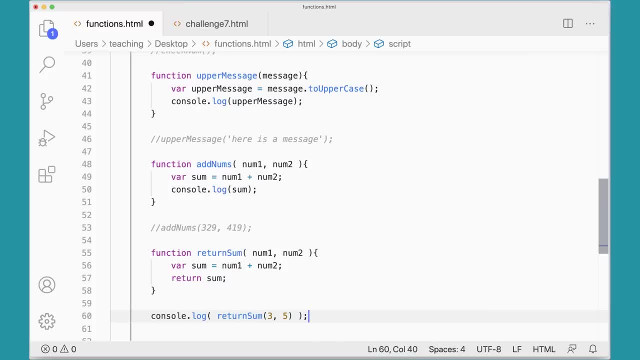 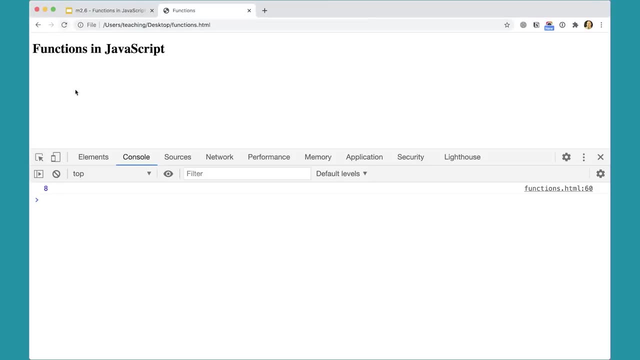 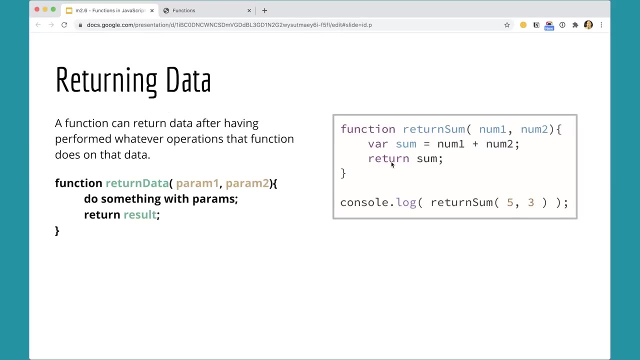 And you'll see when I run this over here, assuming I type that, all right, that in fact I get an 8. And it's still going to the console. So you might wonder, well, what's the big deal here? What's the difference here between returning the sum? 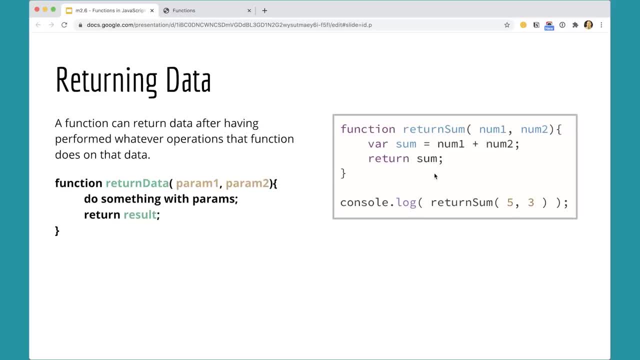 and just having it print out the finished thing. here, The analogy that I like to use is one where you're washing your clothes. If you happen to have a washer and a dryer, you have two machines And those machines work together, So you put your dirty clothes in the 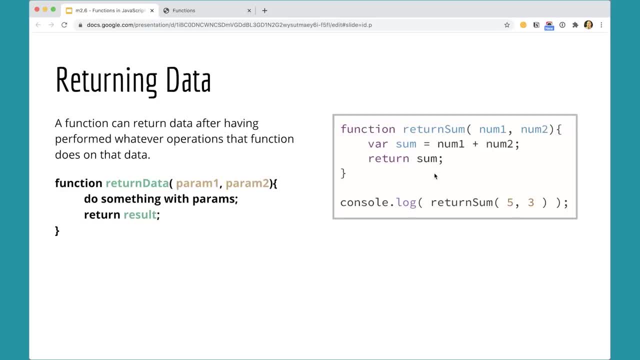 washing machine. So you're feeding it in dirty clothes, dirty laundry, And you're putting in soap and you're putting in water, And the washing machine agitates it all and runs it all together And what it returns to you are clean, wet clothes which you then put into a dryer, And the dryer 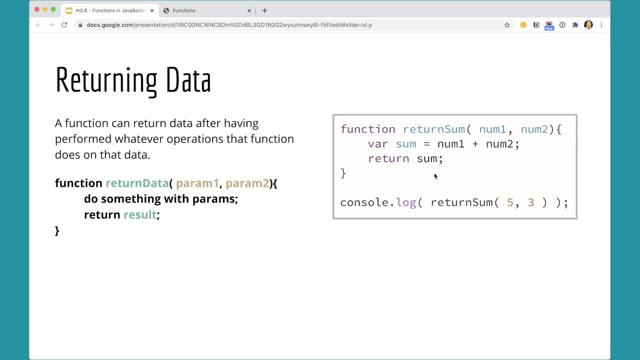 will then do its function, Which will tumble the clothes with air- hot air maybe- And then return to you clean, dry clothes, So you can think of returning as a machine doing something and processing something, doing something to it and then returning the result to you so that you can then 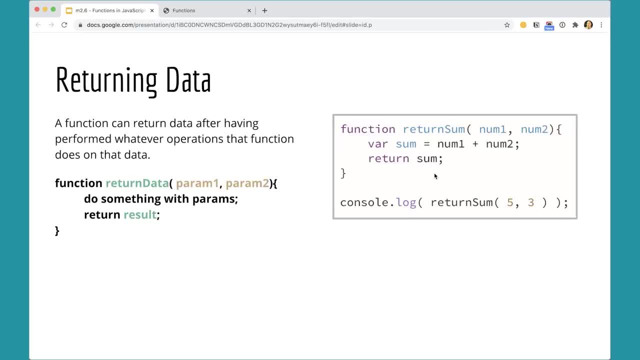 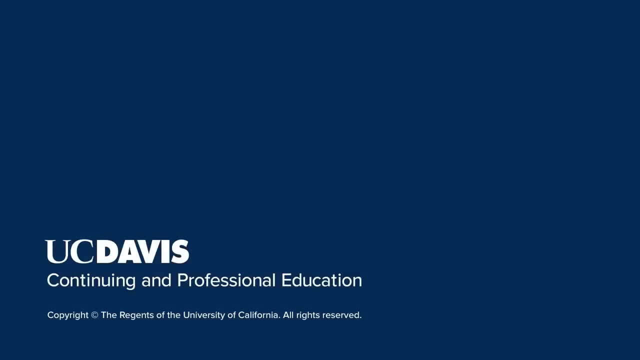 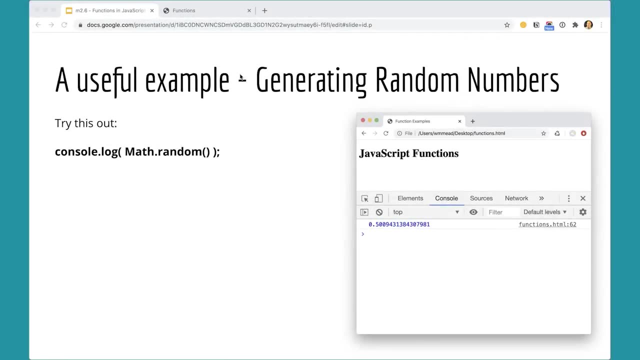 turn it over to another machine that has its special features and does what it needs to do. Let's take a look at a useful example. This will show us something that a function can do for us in JavaScript right now and that we could use in some programs that we write And that is for. 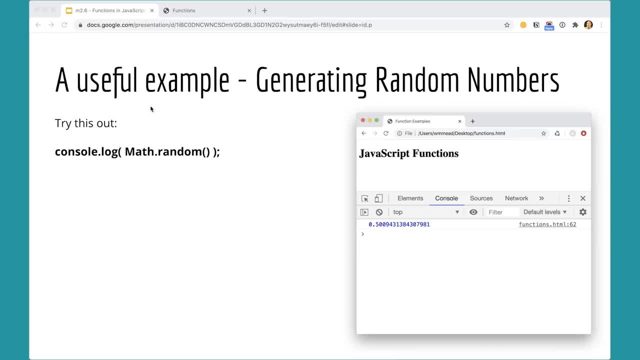 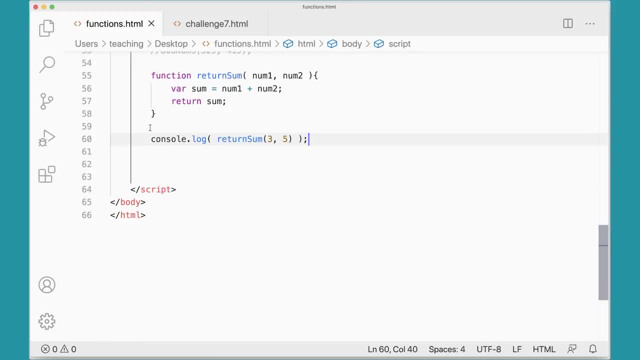 generating random numbers. Try this out. JavaScript has a random number generator And I'm going to just give this a try. I'm going to go over here on my file. First of all, I'm going to comment that out. So I'm not getting that, But I'm just going to. 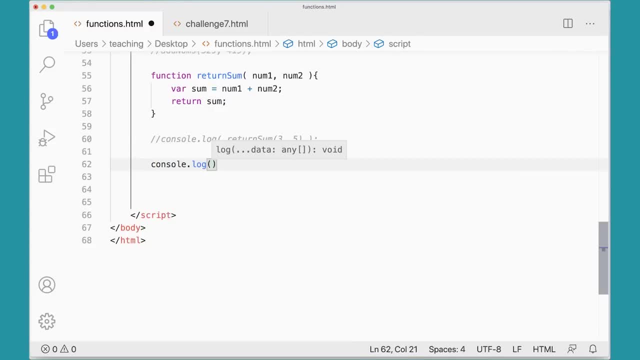 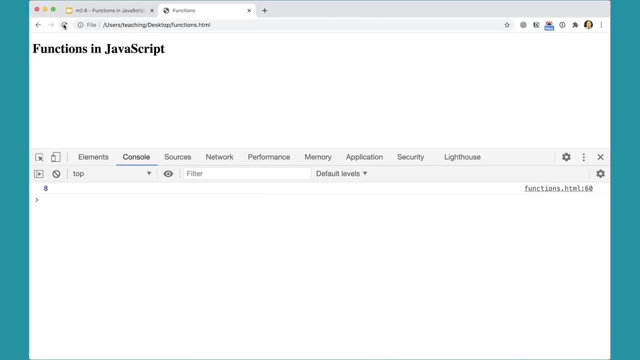 consolelog math with a capital, M, dot, random, And we'll talk more about what that means in a little bit. But math random is going to generate a random number. So now if I go over here to my browser and run it, you see that I get a number And I can keep refreshing my screen. 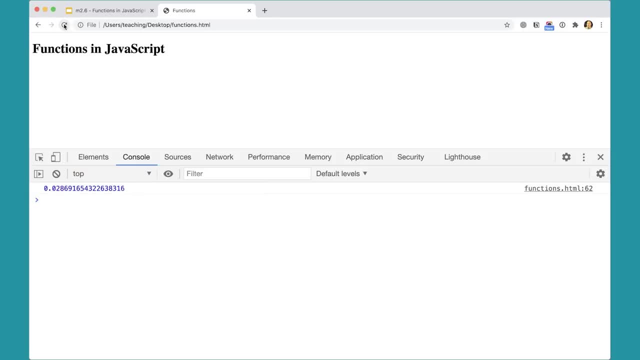 and I'll keep getting numbers. The numbers that I get will be from zero all the way down to 0.0000000000 zero all the way up to almost one. You saw a minute ago I got a 9.9, something or other. 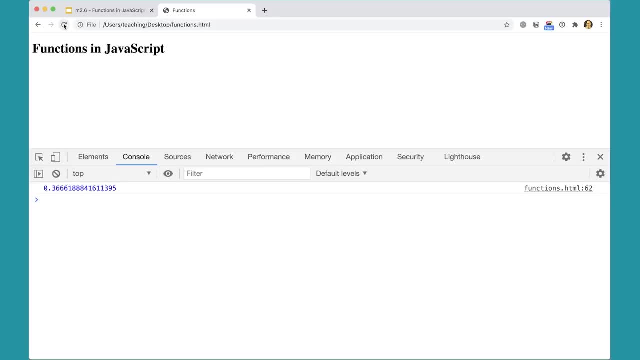 So it won't go all the way to one. You saw a little detail, it's very nice. So it's going to go to not up to 0.9999999999999999, something like that, But it won't go all the. 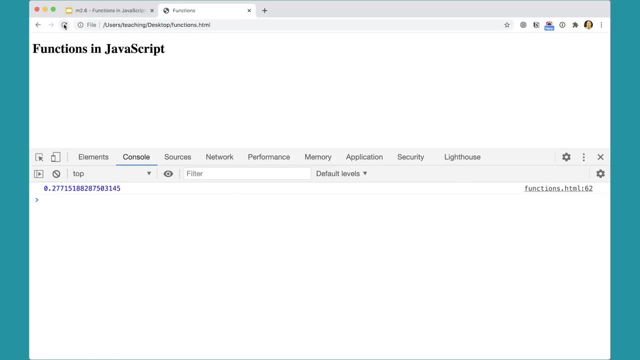 way to one. It could go all the way to zero, But it won't go all the way to one, But it's somewhere in there. So what if I wanted random integers? What if I wanted to get a random number between, say, 10 and 52 or something like that? How would I do that? I need to 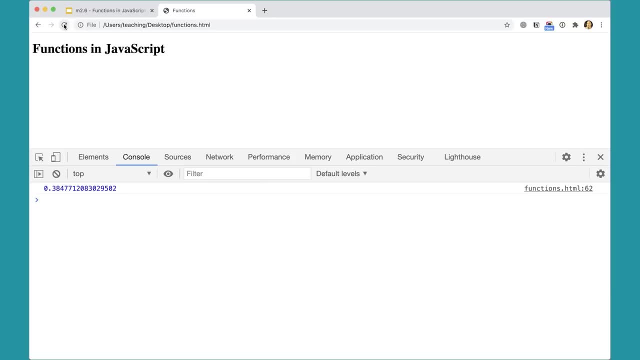 write a function to do that in JavaScript, because the random number generator in JavaScript generates random numbers between zero and almost one Zero, inclusive one exclusive. That's the way that's officially said. So we can see that that's what's going on here. But if I was playing a game of cards and I had numbered my cards, one, 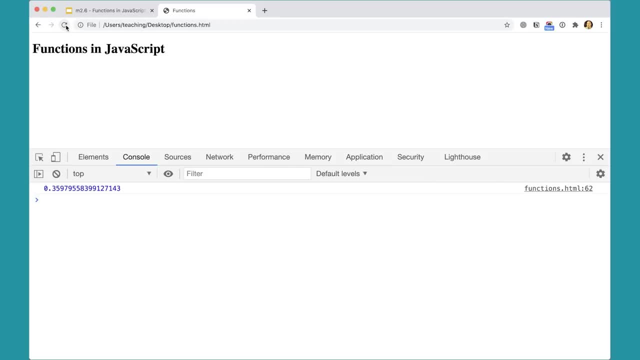 through 52, and I wanted to make sure I could pick a random card. I would need you know to be able to pull out a 26,, not a 0.35979558399127143.. That's not very helpful. 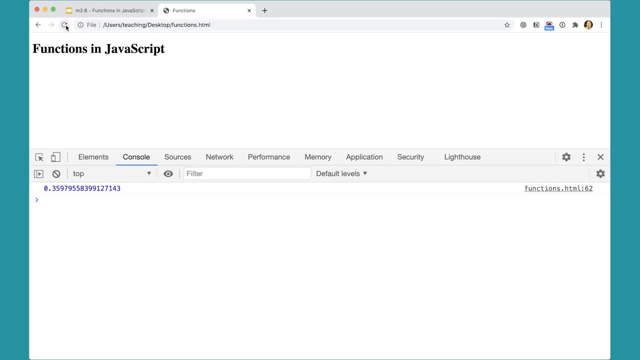 So I need to figure that out And, before we go forward with this, I should mention that the random number generator in JavaScript is not truly random. It's using an algorithm to generate the random number And it's random enough for our purposes, but it's not a truly random number. 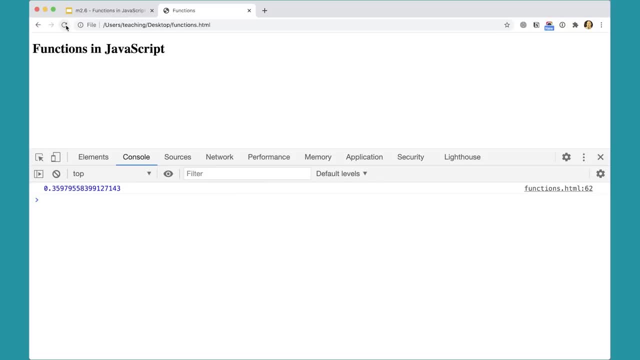 And if you are, If you were making a game that was, you know, making a program that really needed to be random, like a lottery generator or something like that- you would want to use something other than the built-in random number generator, But for our purposes it's random enough, So that's worth. 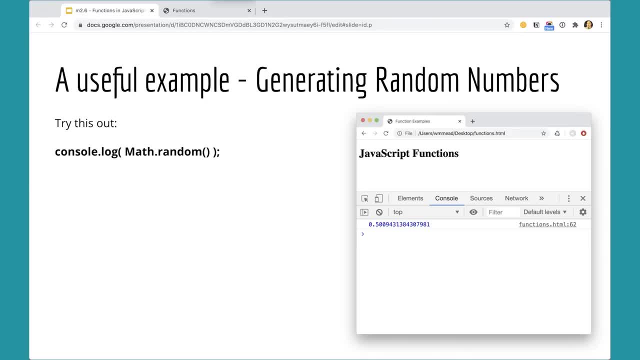 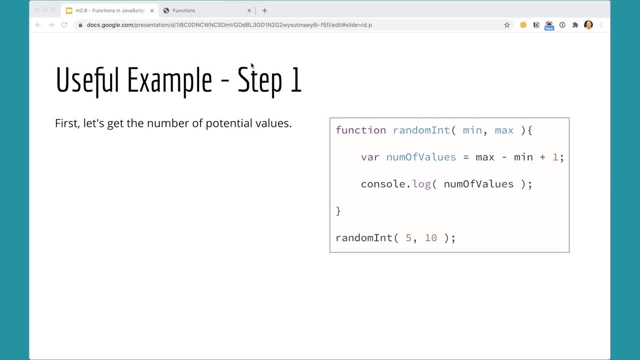 mentioning as well. Here's our first step in creating our random integer generator is we're going to make a function called random int And we're going to pass in a minimum number that we want to get and a maximum number that we want to get. 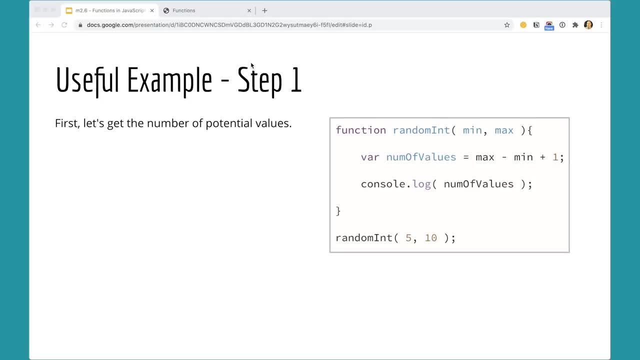 in our random integer generator And to start with, we need to know how many values we think we should be able to get. So I'm going to make a variable called number of values And it's going to take max and it's going to subtract min and it's going to add one to it, So think. 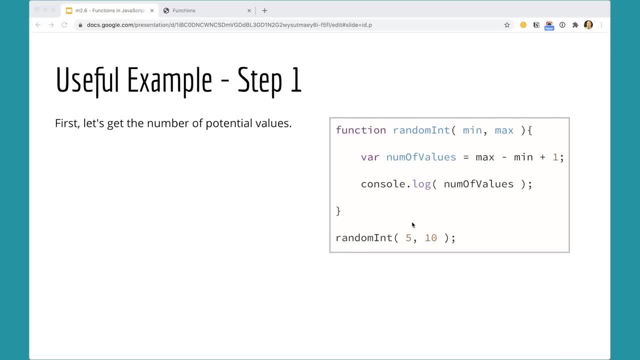 of it like this: If I were to run this function with five and 10, if I wanted to get a random number that was between 5 and 10 and included 5 and 10,, the numbers I could get are 5,, 6,, 7,, 8,, 9, and 10.. That's six. 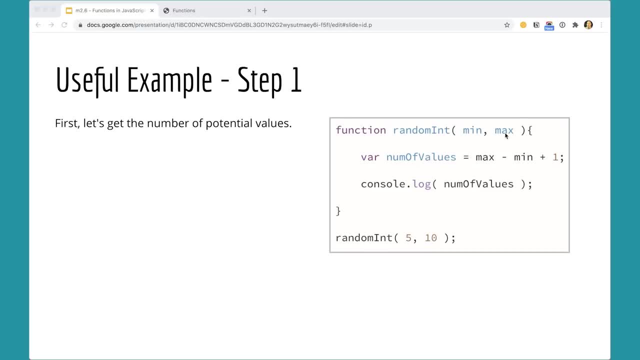 possible values. So if I take the maximum, which is 10, and subtract 5,, that gives me 5 plus 1, that would give me six possible values. So that's how this actually works. So let's go ahead and go. 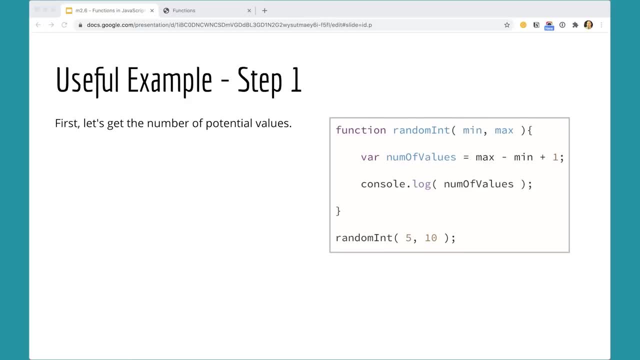 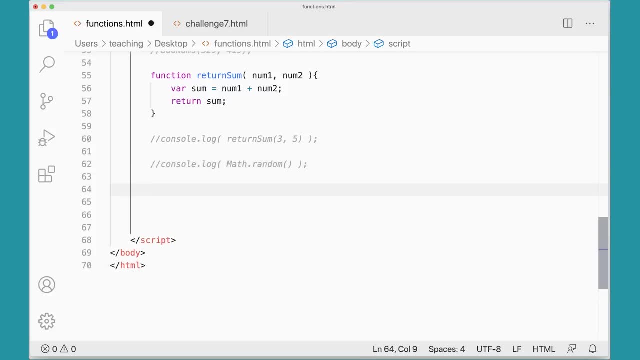 over to our code editor and start writing this function Here. I'm going to comment that out. I don't really need that at the moment, But I'm going to make a function called random int And it's going to take a min and a max And I'm going to have a. 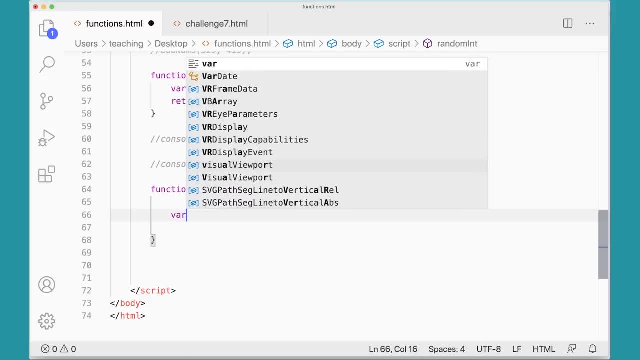 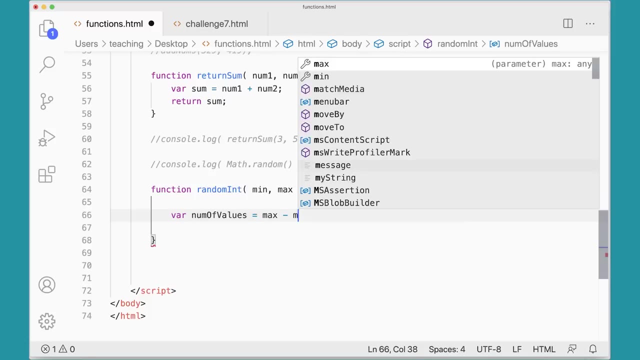 I'm going to have a variable here, bar num of values, And that's going to be the max minus the min plus 1.. Like that, There we go. That looks nice, Okay, great, And then I can just console log out this: 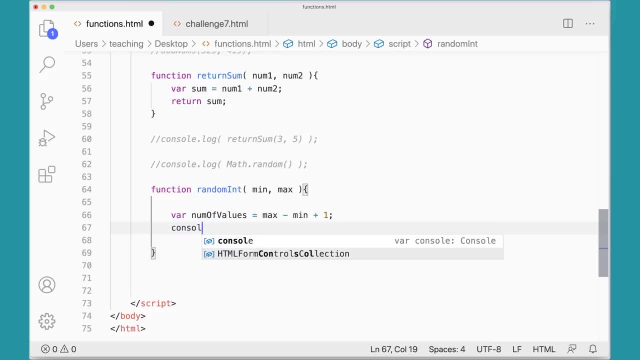 number of values just to make sure it's working right. Console dot log. And when you're working programming you want to do this. you want to just check everything as many places as you possibly can, just to make sure you're getting what you think you're getting. Num of values. So I'm going 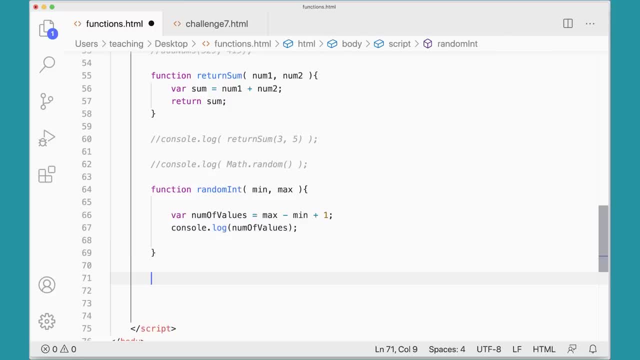 to console, log that out And then down here I'm going to run this function, random int, And I'm going to put in a 5. And I'm going to put in a 10. And we'll see we should get a 6.. 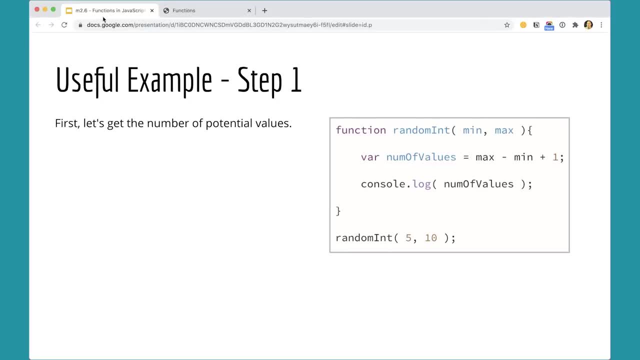 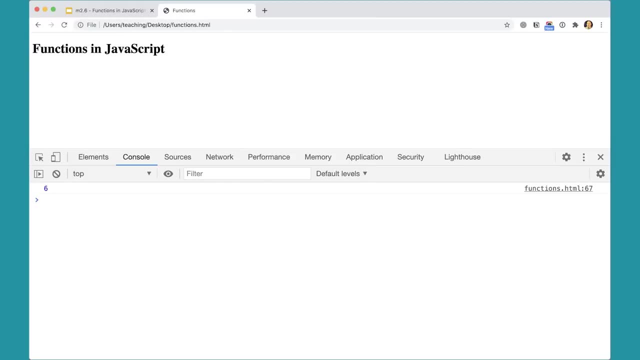 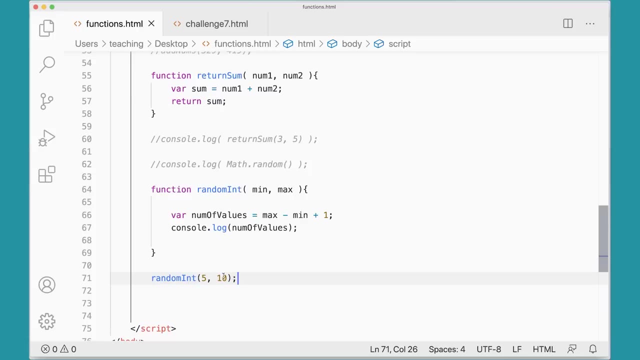 Right, That's what we should get. So let's go over and check that And, sure enough, I'm getting a 6.. Because the possible values if I'm going to include, if I'm going to say I want random numbers from 5 to 10, I want to include 5 and 10.. So I'm going to 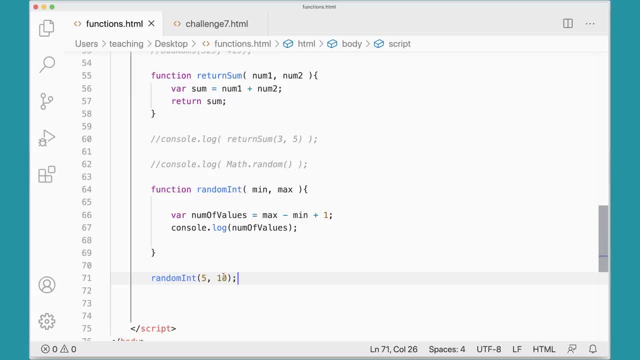 I could get a 5,, a 6,, a 7,, an 8,, a 9, or a 10.. That's 6 possible values. So step one of this is correct, And then we'll go on from there to the next step. 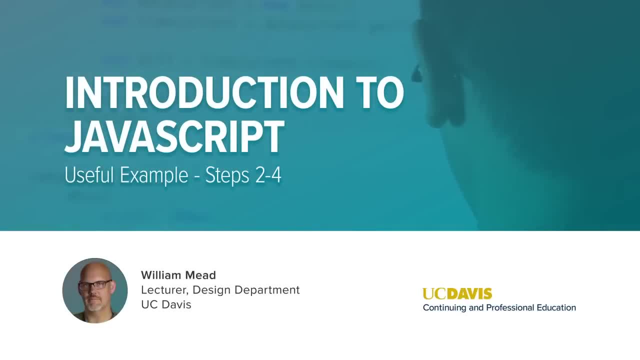 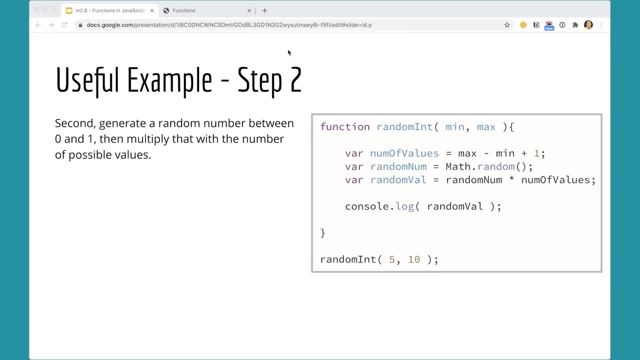 In the second step for our random integer generator, I'm going to actually generate my random number, And so random num here is going to be between 0 and 1. And I'm going to take that and multiply it by the number of values and see what I get. So let's go ahead and add this to: 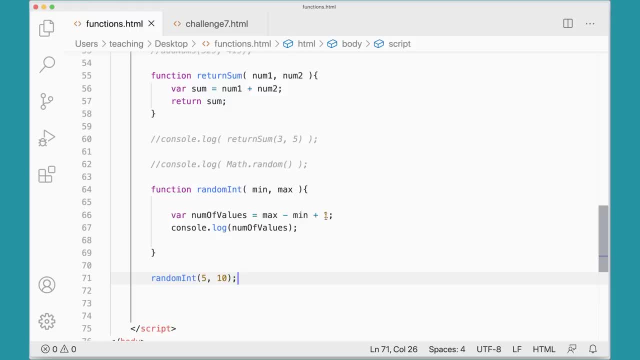 our function over here. So we've got that in there. We can get rid of that. We can get rid of that. We know that's working, So we know that's all good. But now I'm going to get var random num and have that equal mathrandom. So that's going to generate my random number. 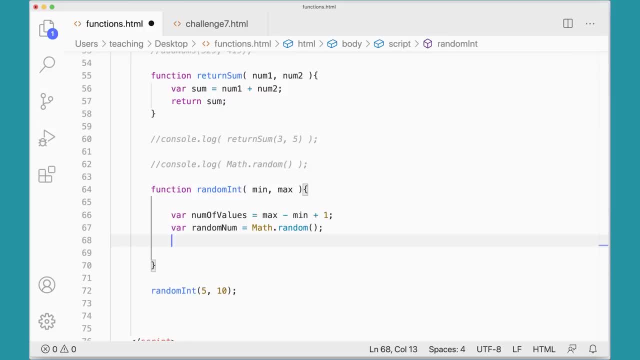 And then I'm going to say: what did I name this variable over here? I've forgotten already. Random value, Random val. I'm going to take var random val and have that equal random num times number of values, And let's just see what that. 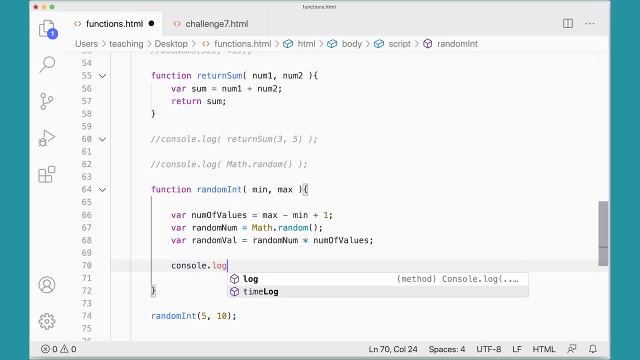 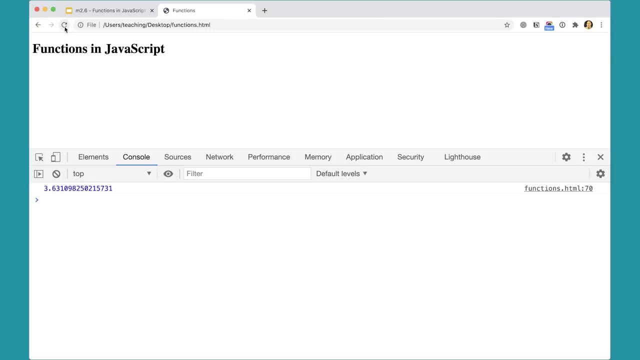 gets us Consolelog random val. Try that out. Let's go over here and run that, And now that's getting me numbers that are between 0 and 6. It won't go all the way up to 6.. It'll get me to 5 point something or other, but it won't go all the way up to 6.. 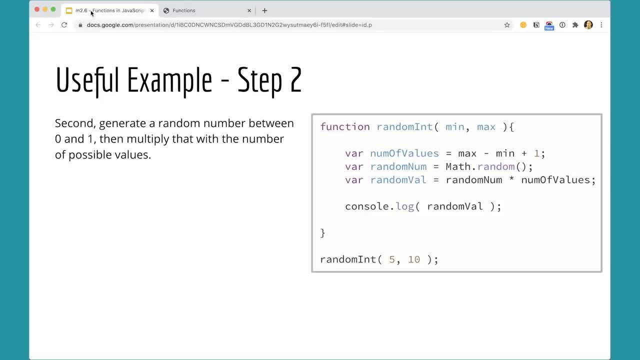 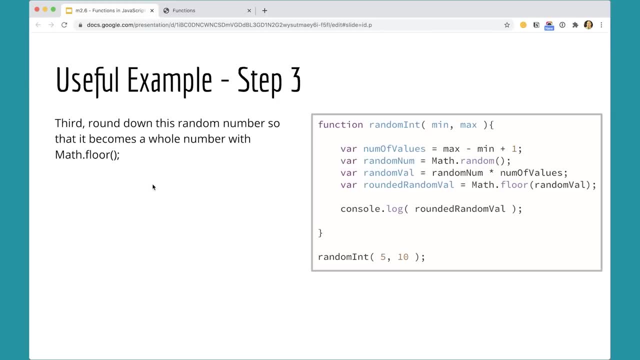 That's interesting. Great, So we're making progress. Let's see what we need to do next. Next, I'm going to use the mathfloor method to round down my random number. So now that should get me a number. that's a whole number, between 0 and 5.. 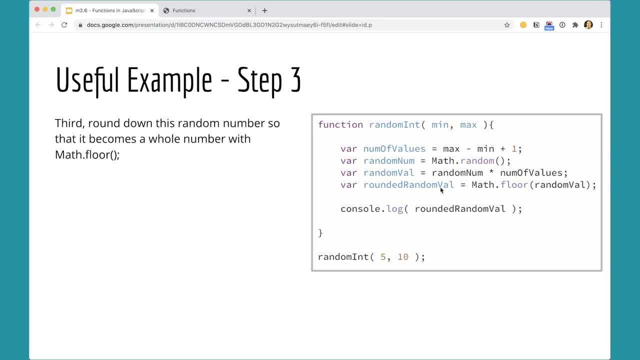 So I'm going to add this variable rounded random value and I'm going to use the math floor and pass in this random value here. This is my number with all the decimal points. So I'm going to put that decimal place is only one decimal point but the number with all the 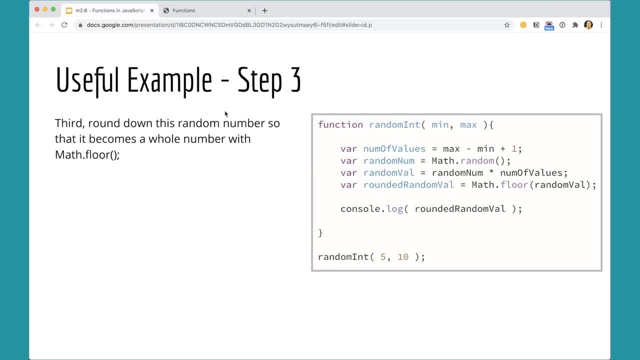 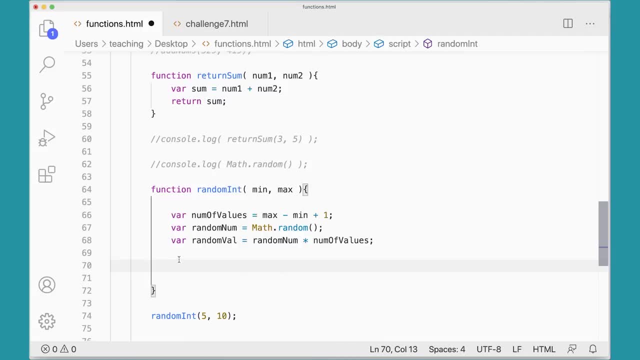 numbers after the decimal point. There we go. That's the way I should say that. Okay, So let's give that a try over here. I'm going to get rid of this consolelog. I don't really need that one anymore, But instead I'm going to do var. 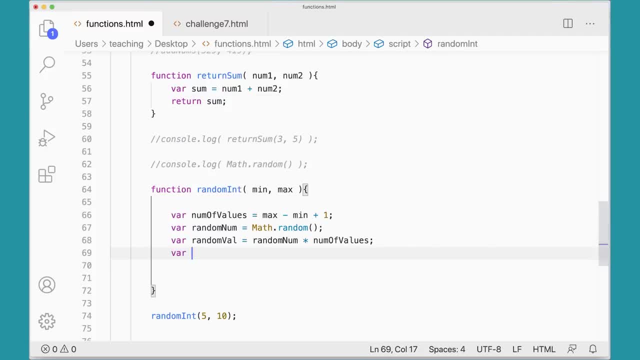 I'm going to do var, rounded, random, Now kind of a long variable name, you can make it shorter. And I'm going to do mathfloor. Floor is a method and seal is a method, Seal for ceiling. So floor will round it down, Seal, 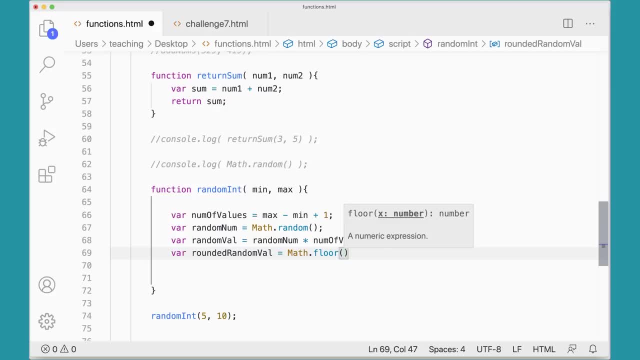 C-E-I-L will round it up Short for ceiling, if that makes sense. And then I'm going to pass in there random value. And once again, just to see what my progress is, I'm going to consolelog, rounded random value. And you saw, I didn't have to actually type that, I just pressed tab, because 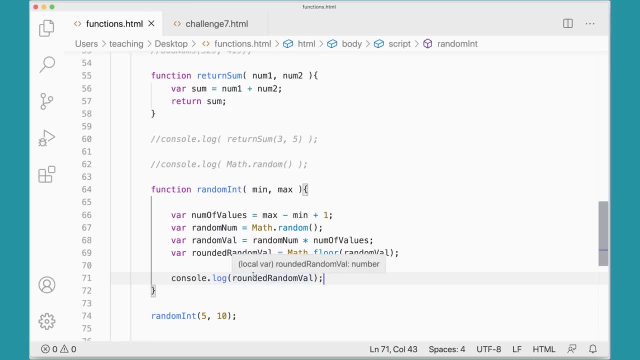 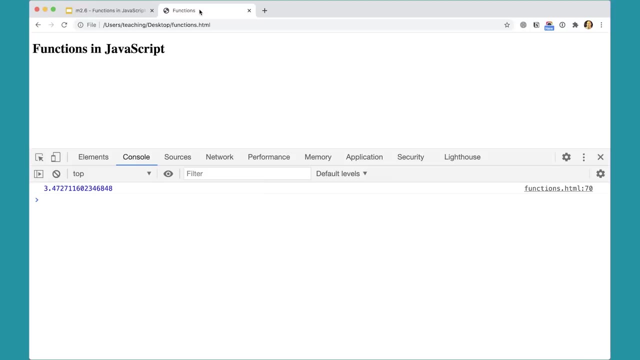 it came up in Visual Studio Code. That'll keep me from getting these long variable names wrong. I could just do RRV or something like that to make it shorter. But that's okay. I'm just making it match my images here so you get a sense of what's going on here, Okay. So now when I run this: 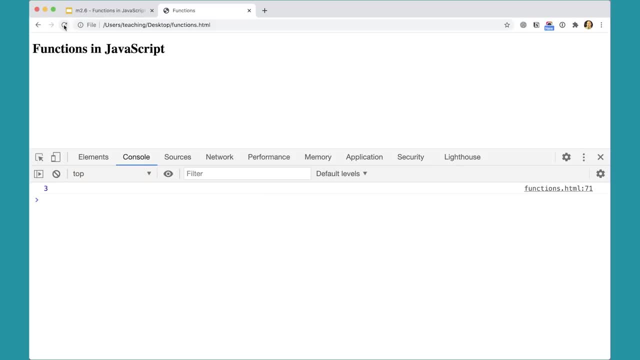 I get a 2.. I get a 5.. I get a 0.. I get a 2.. I get a 3., 5. 0.. So now I'm getting whole numbers, But they're not from the same number. They're from the same number, They're not from the same number. 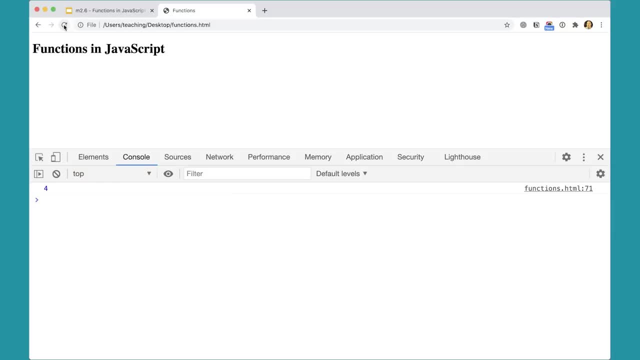 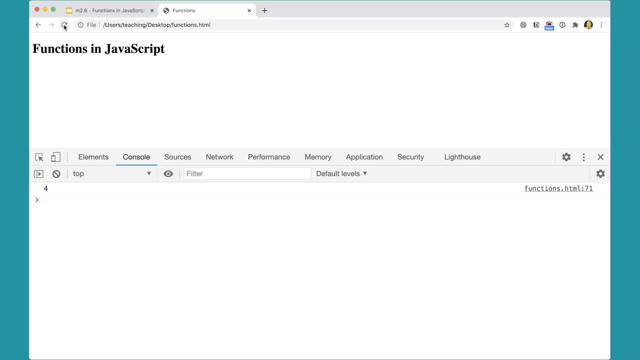 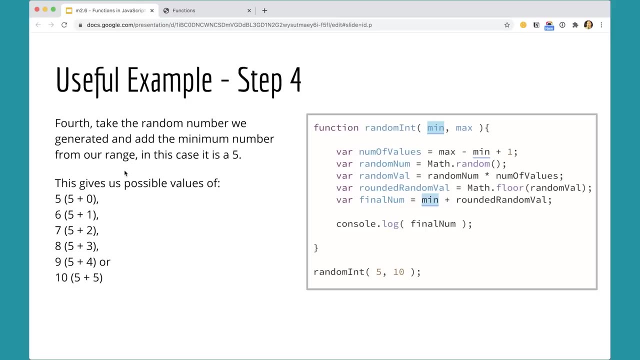 But I'm not getting the numbers between my range that I really wanted. But that's okay, Let's see what we can do next. And now, what we can do next is we can get our final number And we're going to take the min and add it to that range, And we're going to take the min and add it to that range. 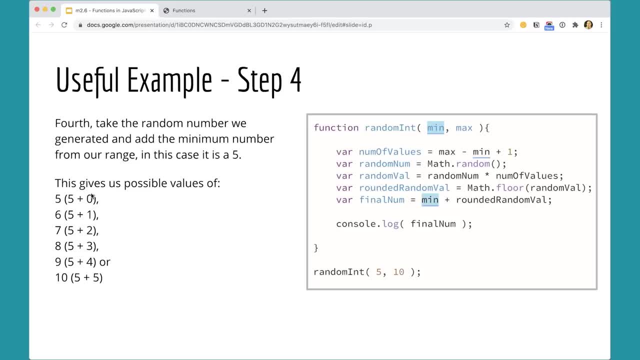 So, for example, if our random number gave us a 0 and we add 5 to it, we'll get a 5.. If we got a 1 and we add 5 to it, we'll get a 6, all the way up to 10.. So that will give us our random numbers between: 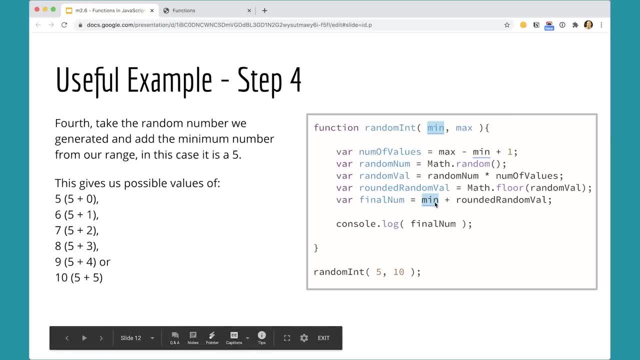 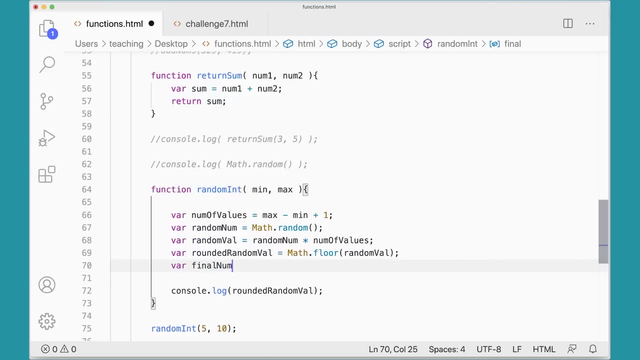 5 and 10 if we add the min value to this final number here. So let's go ahead and add that in there and see what we get. bar final num equals min plus rounded random val And we can console log that out. Come back and 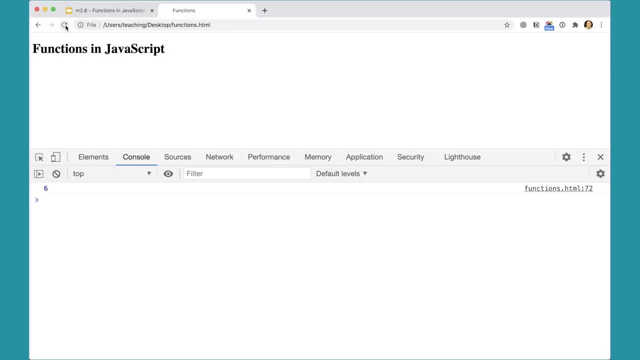 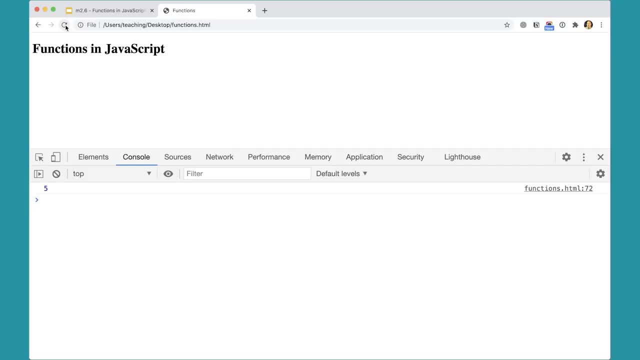 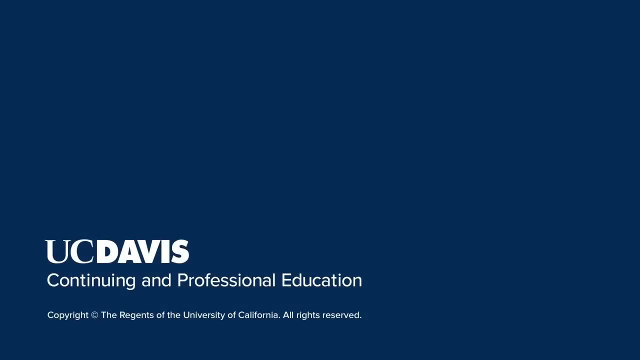 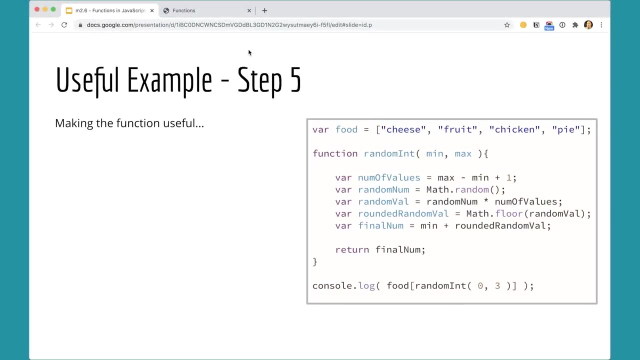 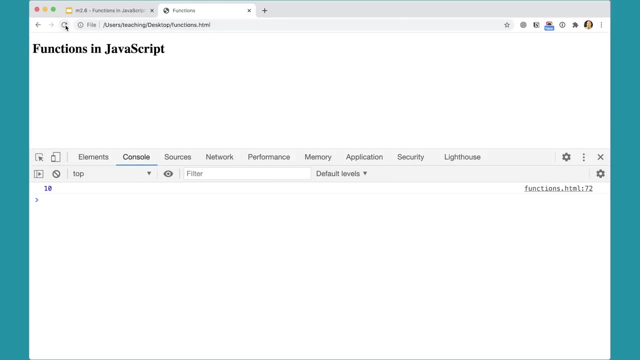 random number generator is actually working, which is great. In the next step, we're going to make our random number generator, our random integer generator, a little bit more useful. Currently it works. We can generate random numbers, But the only thing we can do with these random numbers is see them pop up in the console, which is really. 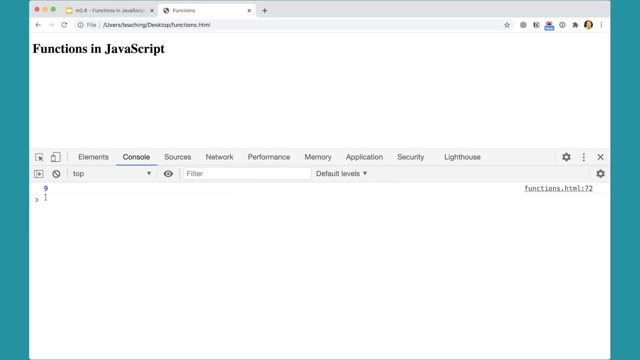 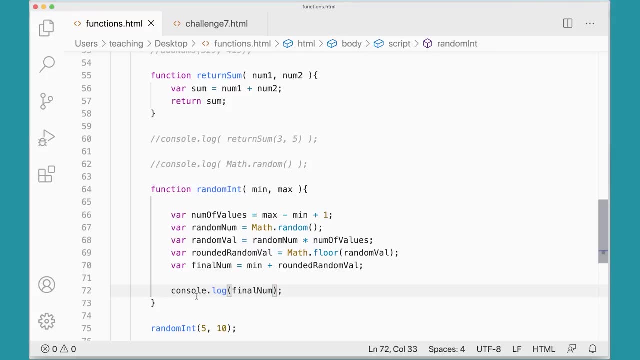 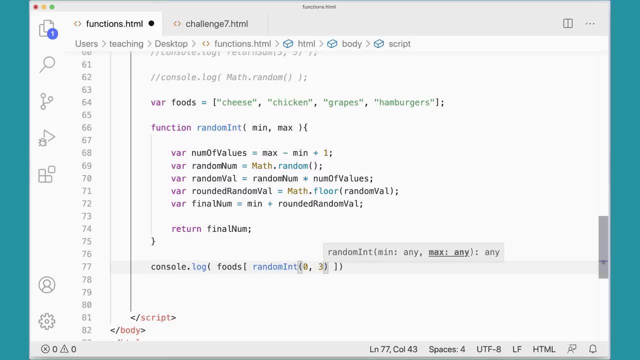 return the number to the console. And we could return the number to the console And we could three. and now, because this random int zero three is going to be, because it returns final number, it's going to be a zero, a one, a two or three. so console log. 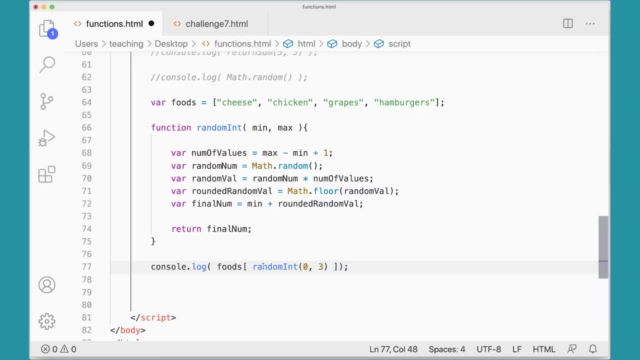 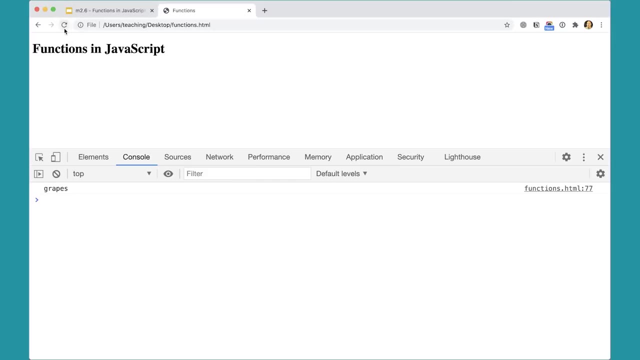 foods: random int zero. comma three is going to go into the array and get me either a cheese, a chicken, the grapes, or hamburgers. let's see if that works. if I typed it right, and sure enough, I got hamburgers and then I got grapes and then I got chicken. so that's working just fine and I can actually use my. 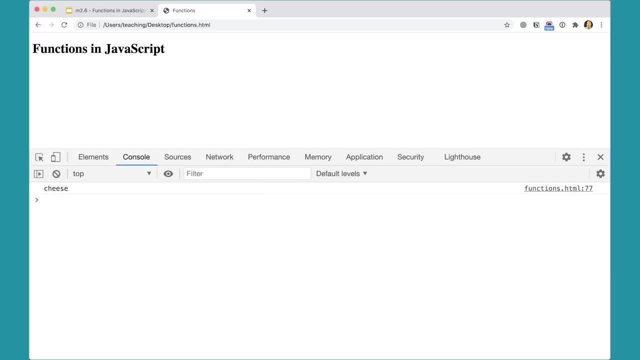 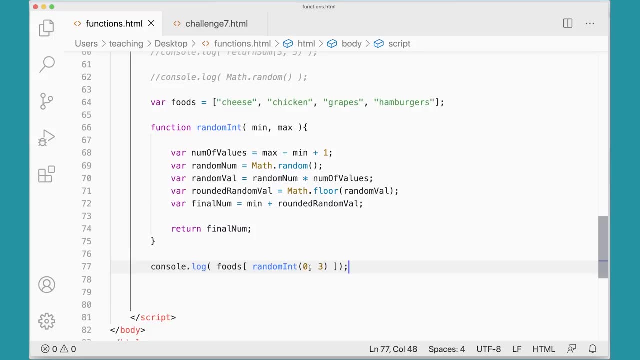 random number generator to actually do something with another program. so you can think of this: because this thing returns a random number, I can use that within my tool here to get something out of this array, and then I can actually use that to get something out of this array and 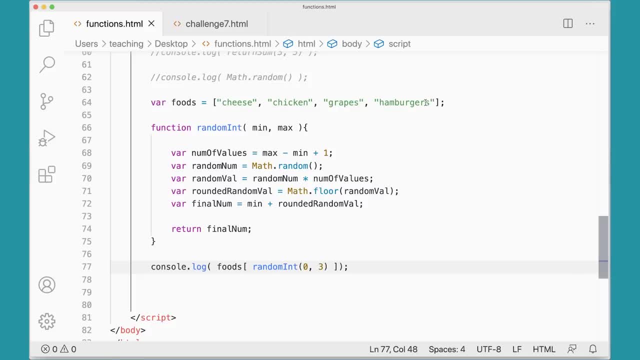 then I can actually use that to get something out of this array. going back to the washing machine and dryer kind of example, this is my washing machine. it's returning to me a process number that I can then. that I can then use with foods to do something. I don't know, it's not that interesting, but it's a little bit. 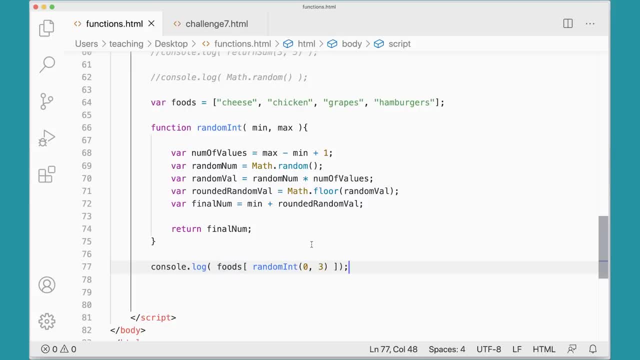 more interesting than what we've been doing so far. okay, great. one last thing to look at and think about for this is that this function is pretty long. we want to refactor it. remember, we want to refactor as much as we possibly can. so what we could do is we can refactor this thing down quite a bit here. what we want. 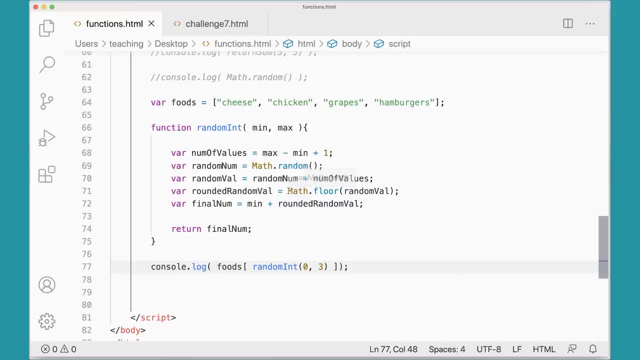 to return is really this math floor random val. so I'm going to take that, I'm going to stick it down here. I select that right. there we go. I'm going to return rand. I'm going to, I'm going to do that, but in here what I'm. 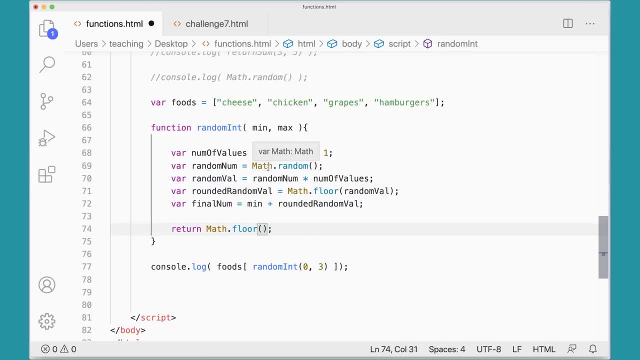 going to take is I'm going to say really, what I want is I want this max plus min. I want to put that in here. I'm going to put that in its own set of parentheses: max min times: my math dot: random. I'm going to do that and then, outside of this, I'm going to add: 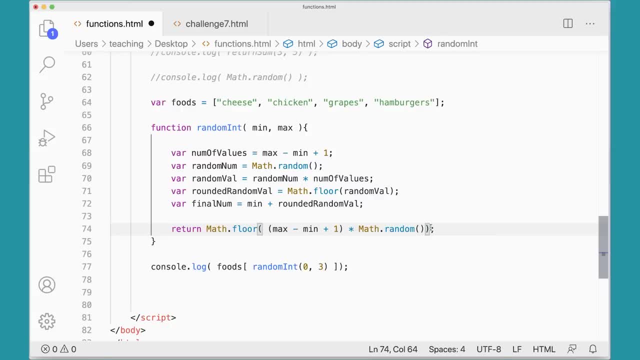 plus. I believe that will work. I think I have that right. let's see if I have that right. I'm going to comment this stuff out for the moment. I'm pretty sure that's right, because I'm going to return, I'm going to take math floor, I'm going 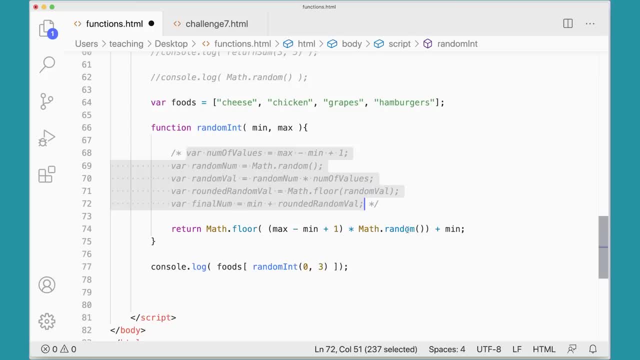 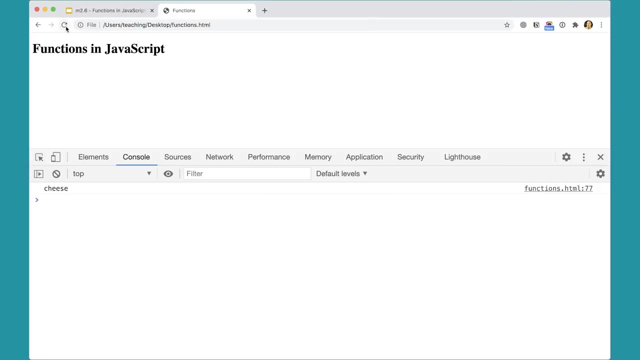 to take my max, subtract my min and add one. multiply that by math random. I'm going to round that down and add min and that should be doing the same thing as this. let's see if I did that right over here. if I run this again, I am. 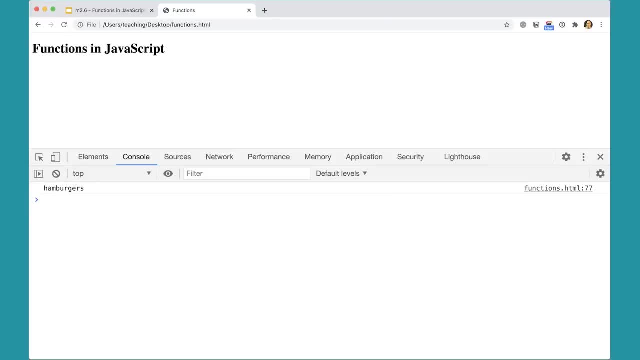 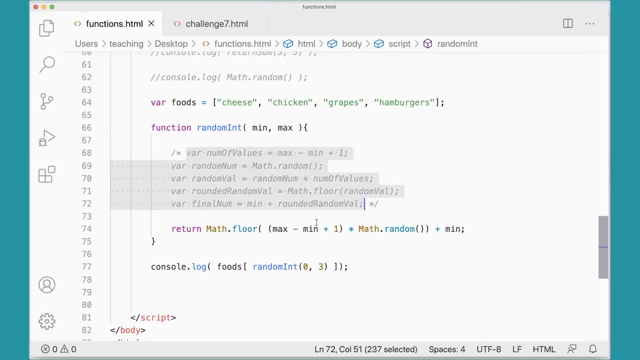 still getting my items here. so this is a shortened version of all of this stuff. now you might look at this and go: well, I don't really understand what's going on here, and that's because I'm going to do that and then, outside of this, I'm going to. 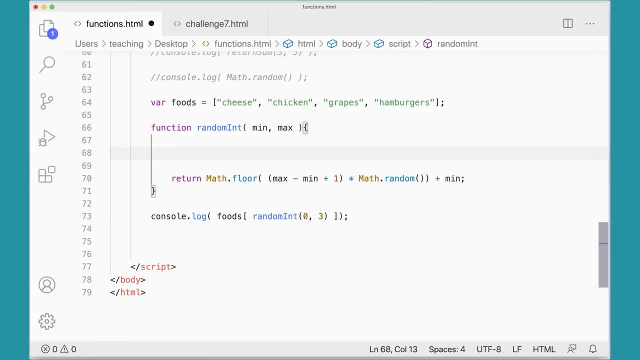 add min and max, and that's a great place for a comment. so here you could say something like you know, creating a random integer- min and max- or you could put a more explicit statement in here. sometimes taking a big line of a big chunk of a code and reducing it down to one line can be difficult to understand exactly what it's doing. 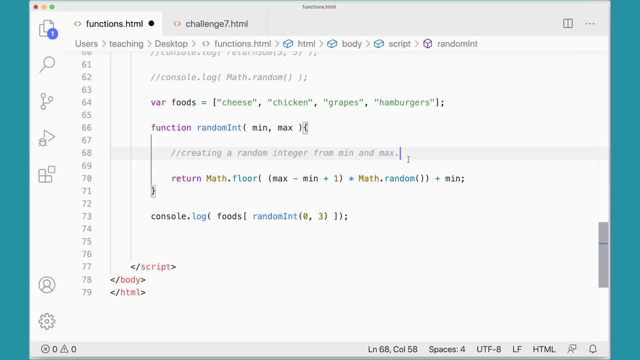 later. But in this case I kind of like it, because if you were to go looking around on the web for random integer generator for JavaScript, if you Google that, you'll get statements that look like this. You'll get functions that look like this. You'll find them on Stack Overflow and other. 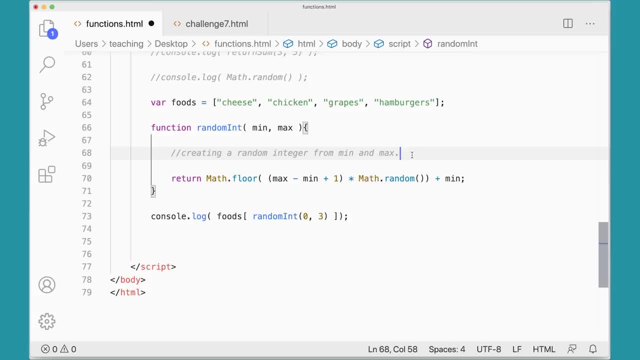 places, So it's kind of useful in this case. Sometimes these one line statements where everything's reduced down, become very difficult to read and understand exactly what they're doing, But I think this one's pretty good, So I kind of like it. Okay, so that allows us to create. 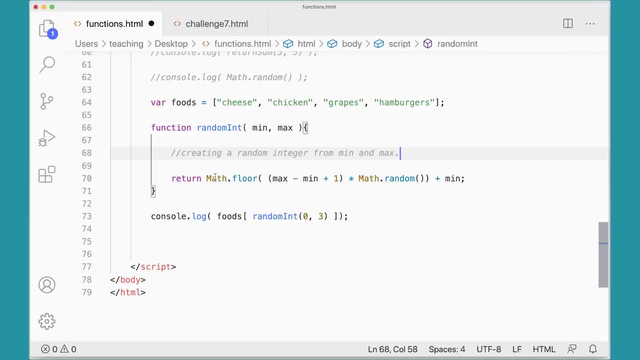 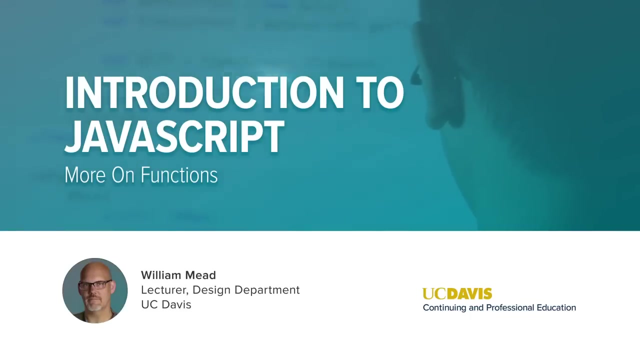 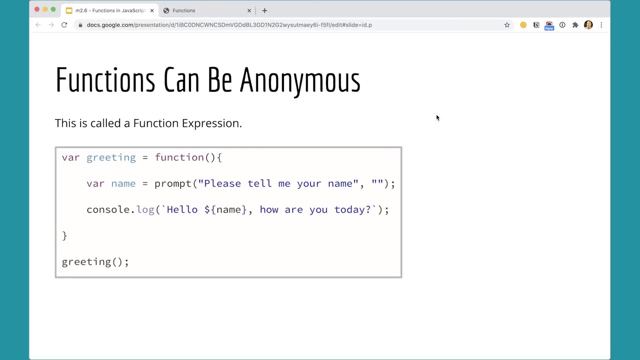 a random integer generator that we then refactor down into one line of code. But by walking through the steps you could sort of see each step along the way And how that actually worked. We have a few more things to talk about in terms of functions before we're done with this lesson. 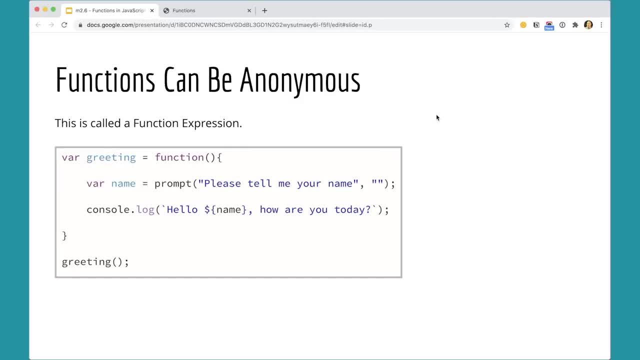 And the next thing is that functions in JavaScript can be anonymous, And one of the important things to understand about the way functions work in JavaScript is that functions are first class systems in JavaScript, which means you can assign a function to a variable the way you. 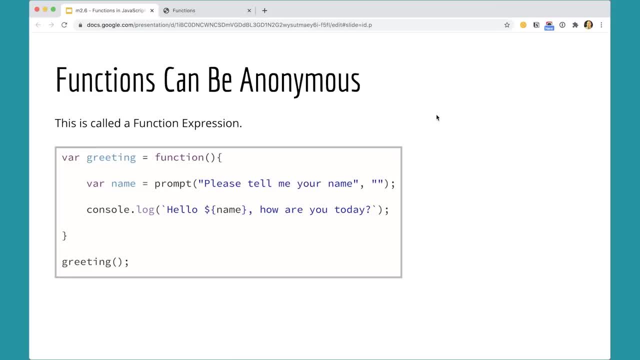 could assign a string to a variable or a number to a variable and, in fact, you can use a function wherever you can use data in JavaScript, and it's one of the very powerful features of JavaScript. if you'll recall, we talked earlier about the fact that JavaScript has some features that are really best in class. 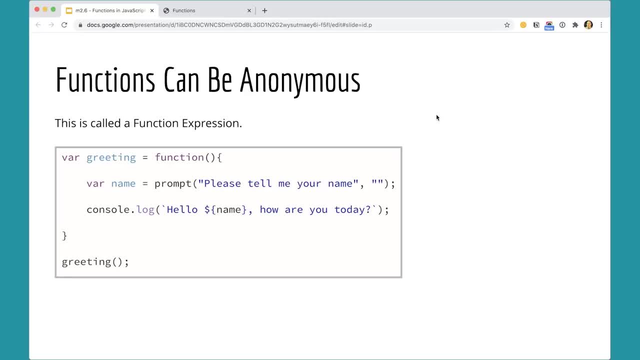 features for any programming language, and this is one of them. this is really a very powerful feature of JavaScript, so you can actually assign a function to a variable and that function doesn't have to have a name. it can be nameless, it can be anonymous. there are times when this is very useful, especially if you're 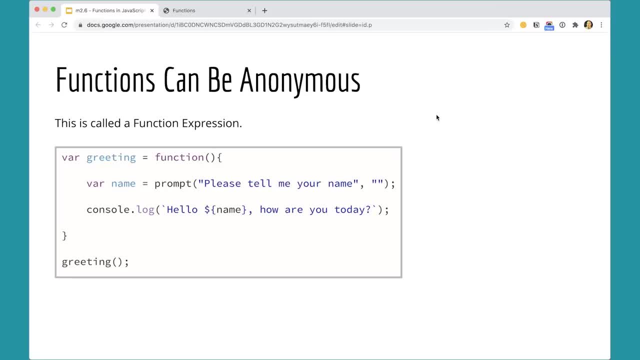 making a function that's really only going to be used once or in one context, then there's really not a reason to create a named function if you're not going to use that name over and, over and over again or in different places in your script. so function expressions are useful for that. they're useful for other. 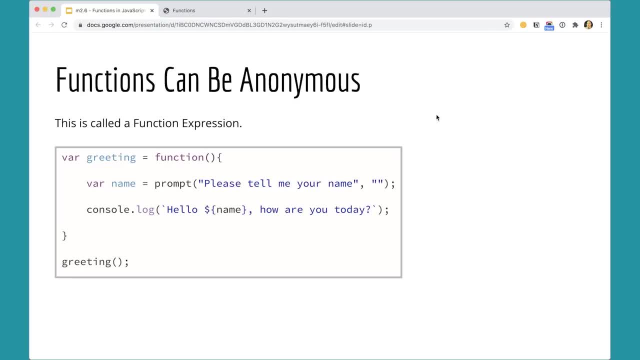 things as we get into more sophisticated JavaScript, but for right now, I just want you to be aware of what they are. we won't be using them much for a while, but eventually. eventually, you'll be using function expressions if you keep working with JavaScript. so let's actually see what this looks like in our 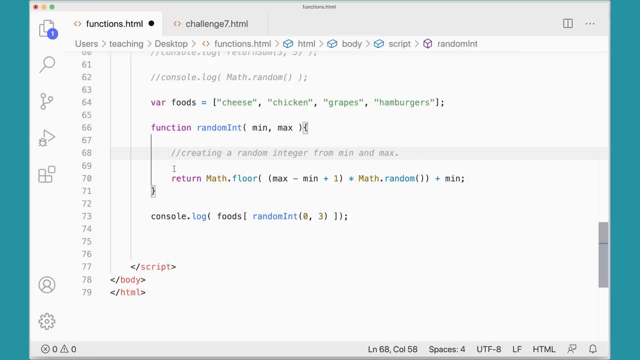 code over here. I'm going to come over to my editor here and I'm going to leave that. that's all fine. but I'm going to make a variable called greeting and I'm going to assign it a function, and you'll see that this function doesn't have a 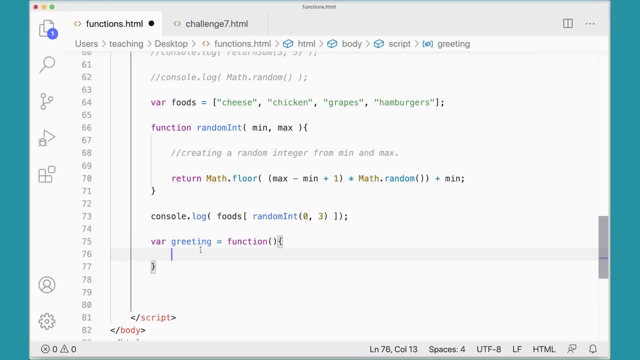 name. it's just an anonymous function and you know we could do whatever we want in here. we could. I'm going to, just for right now, just do consolelog. hello from the function. my slide has something a little bit more sophisticated on there, but for right now this will just do for us, just to sort of. 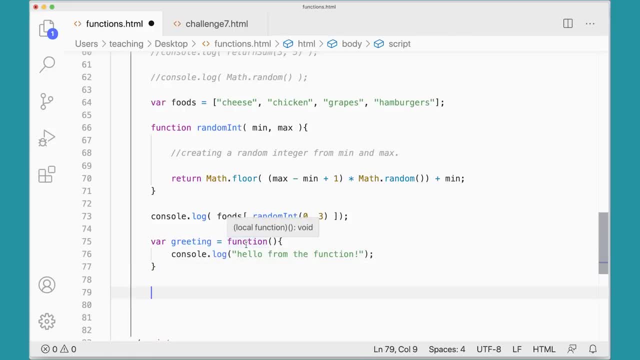 see what this does- and then, in order to call this function- again, remember, we have to invoke the function, we have to call it or run it. I run greeting as if it were a function, which seems kind of weird, but that's the way it works in JavaScript. 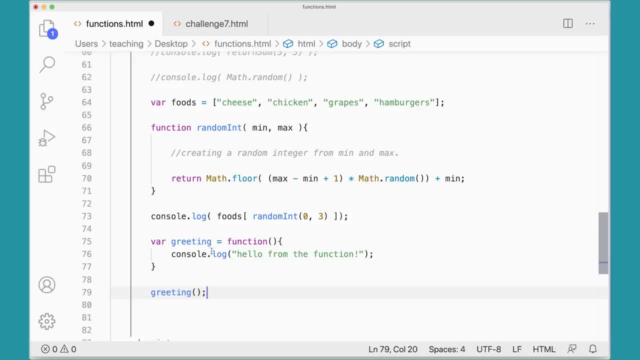 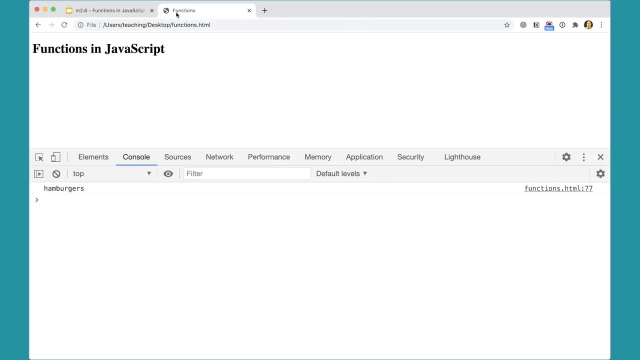 greeting parentheses. so we run that like a function. and now if I come over to my console over here and run this, I'm getting hamburgers again. then I'm getting hello from the function, hello from the function. so that function is actually running. so that's kind of important to understand. 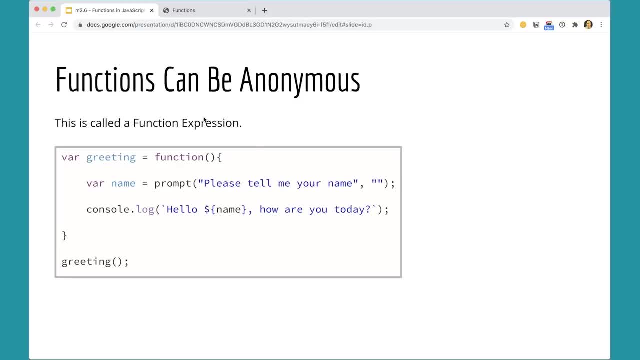 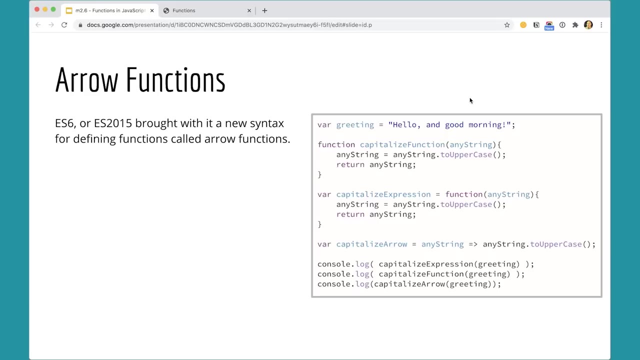 you and again. this is called a function expression, and it's because functions are first-class citizens in JavaScript that we're able to assign a function to a variable just as if it were data. the next thing to understand about functions in JavaScript- and I'm not going to demonstrate this now, but I just want to- 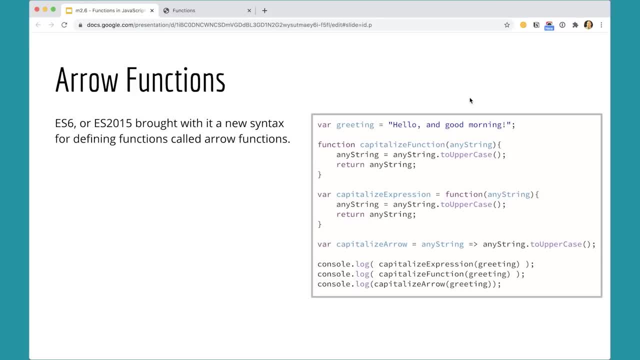 call your attention to it because if you're looking on Stack Overflow or if you're looking up scripts online and seeing other kinds of things, you will see arrow functions, and this is again part of ES 6 or ES 2015. that brought this new syntax and we'll come to it, not in this course, but in the third course. we'll 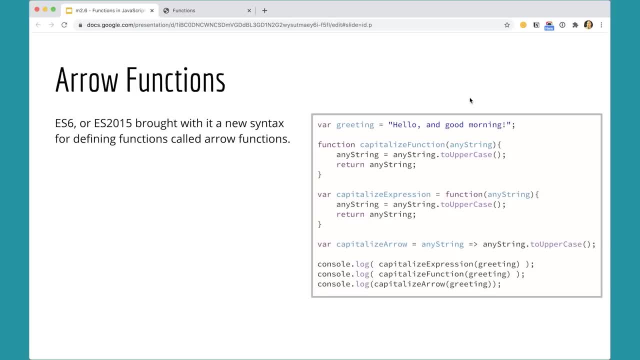 actually start working with arrow functions, but I want to mention them now because you'll see them around and when you look at them, you'll look at me and go: what's this? we haven't done this in JavaScript yet, so I just want you to be aware that it's just a slightly different syntax for writing functions. 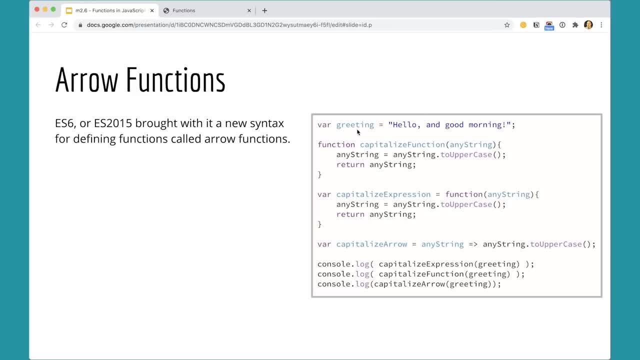 so here I have a that should look fairly familiar. I've got a greeting, hello and good morning, and then I've got function capitalize and I'm passing in a string and then I take that string and uppercase it and then I return any string. So this function is going to return this string. 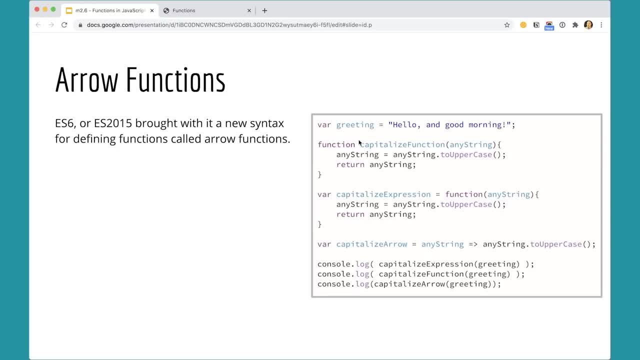 uppercased, And this is fairly- should be fairly- familiar from doing this lesson so far. We've seen this kind of thing and that's not too different from what we've seen. Whereas here we're using the function expression, I have a variable called capitalize expression. 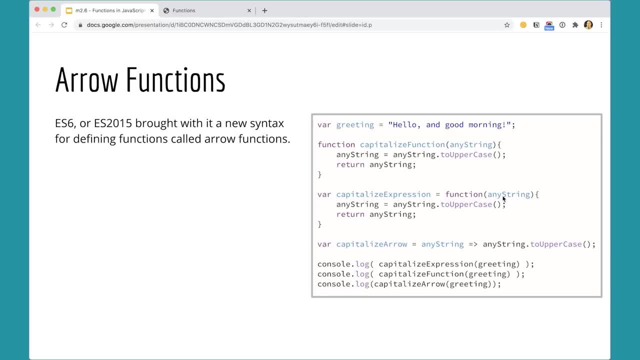 and that has an anonymous function that takes a string and then it takes that string and makes it uppercase and returns it. So this variable will become the uppercase string that gets passed in when it's run. And that's the variable expression, the function expression that we saw just. 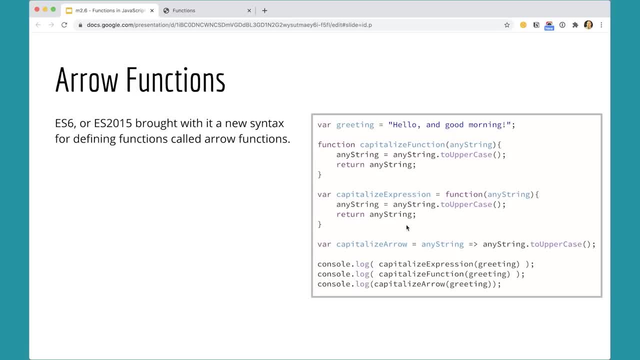 a few minutes ago, When we use the arrow functions- the arrow functions is a different syntax for a function expression And in fact sometimes they're officially called arrow function expressions- So we can make a variable capitalize arrow in any string and then instead of the word function we can just put in this: 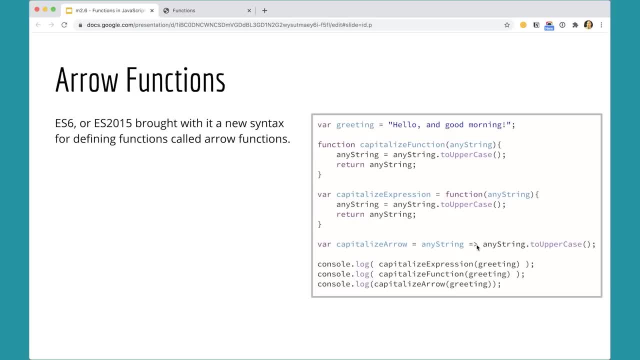 equal sign and the greater than sign to make an arrow And it'll take any string and we can take any string in uppercase and return that. So this becomes like one line, which is one of the reasons why these arrow functions have become popular. is they really do? 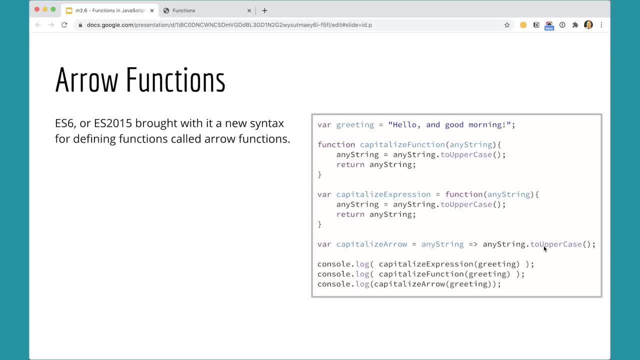 kind of lead to shorter code and less syntax to have to deal with, Although when you look at them it can be a little bit harder to understand exactly what's going on here. But all three of these functions are actually doing the same thing. They will all return. 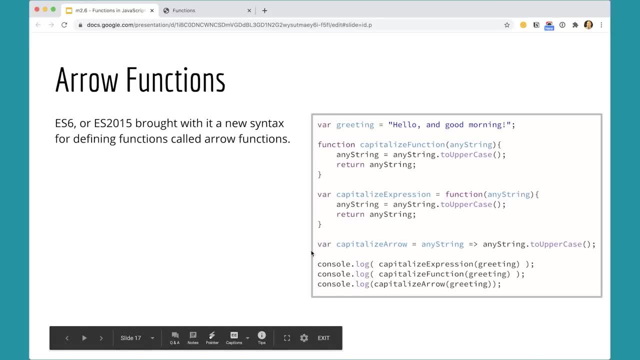 exact same data. so that's kind of an important thing to understand. and again, we'll get to the arrow functions later in the third course, but for right now I just want you to be aware that they exist and that really they're just a different syntax for writing functions, the last thing that we need to talk. 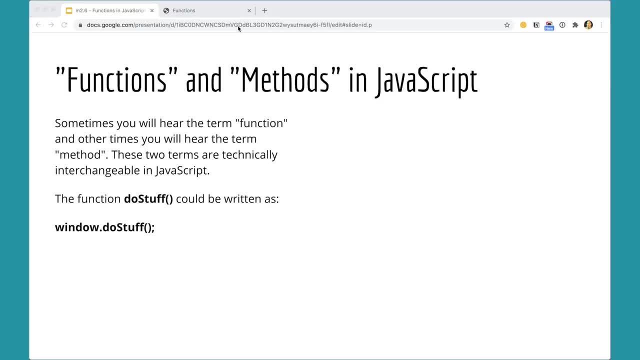 about in terms of our lesson today on functions, is the difference between functions and methods in JavaScript. it can be a little bit confusing because these two terms are basically interchangeable in JavaScript, and you'll you've already heard me use the term method sometimes and functions other times, so it's helpful to know a little bit about what the two terms mean. 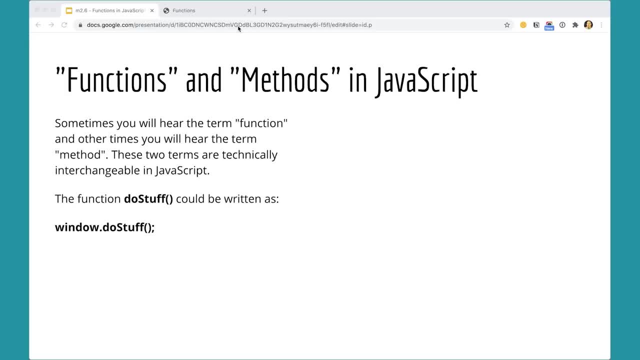 and why they're interchangeable. essentially, in JavaScript, when you have a function that belongs to an object, it's called the method. so, for example, we have the string object and there are functions that belong to string objects, like two uppercase or two lowercase, and when we have a function like that, that 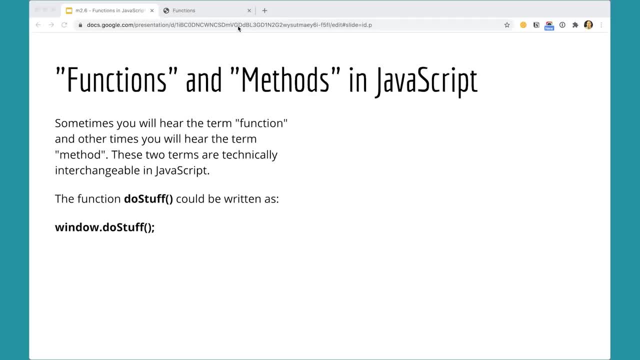 belongs to the string object, it's called the method, it's called the two uppercase method because it belongs to the string object. or another example: with arrays, we have the push method, which is a function that belongs to the array object. okay, so when we push something into a ray, we're using the. 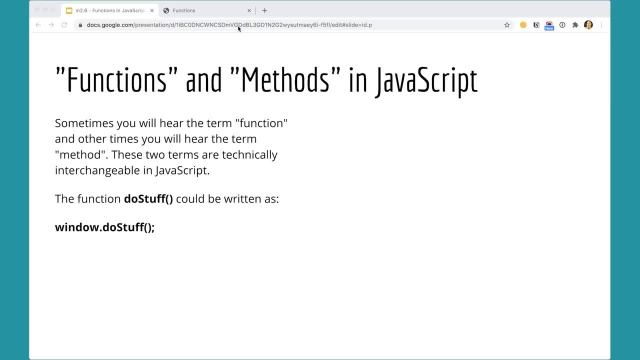 push method and for that. Now, in reality, in JavaScript, everything is an object, So in that sense every function belongs to an object of one sort or another. And in fact, early on in this lesson we wrote a function called doStuff, But doStuff, since it doesn't explicitly belong to some other. 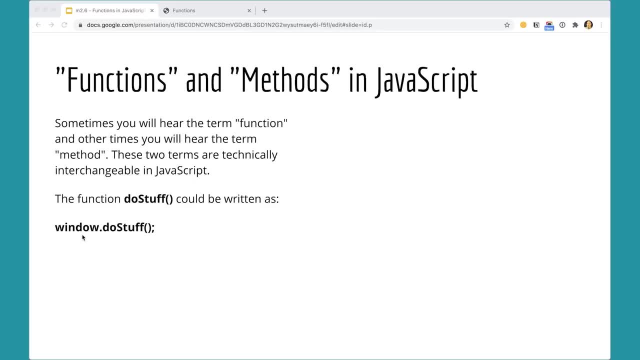 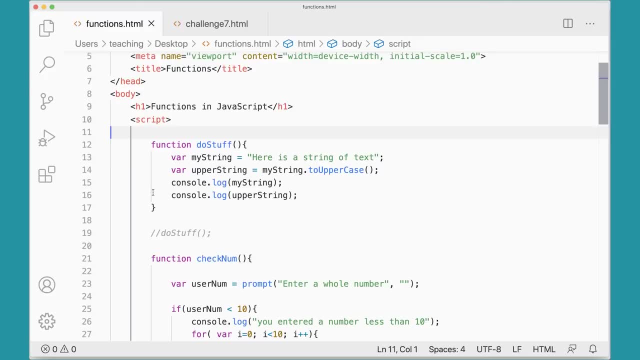 object. it does belong to the window And you could actually write windowdoStuff and that will actually work. So if we go back to our code here and I come in here and I uncomment out this thing and I put windowdoStuff, you'll see if I save that and come back and test. 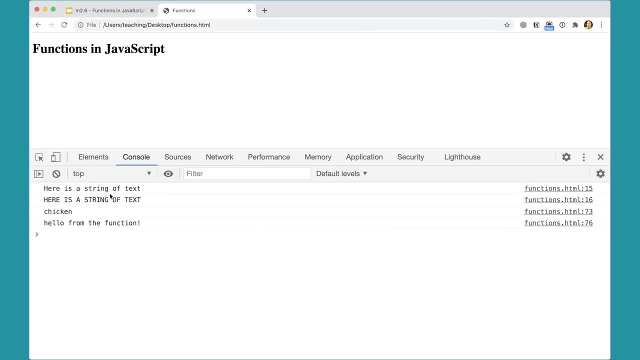 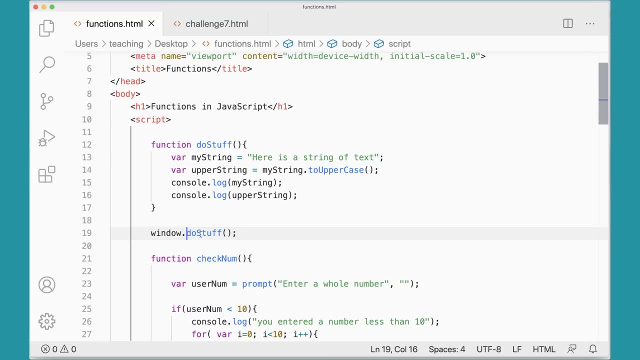 it over here. it actually functions Because ultimately my doStuff function belongs to the window object. Now, we don't often if a function belongs to the window object. we don't often do this. Occasionally we do, but very rarely will we put windowdoStuff in there, We'll just call. 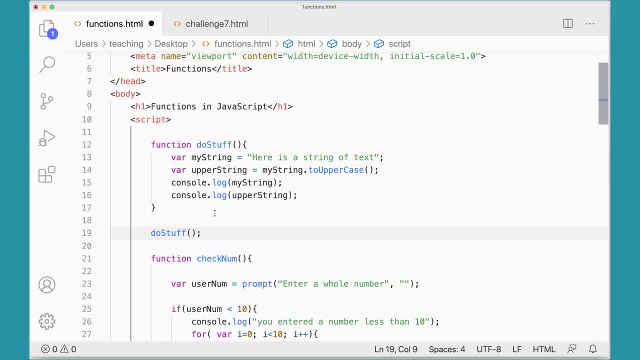 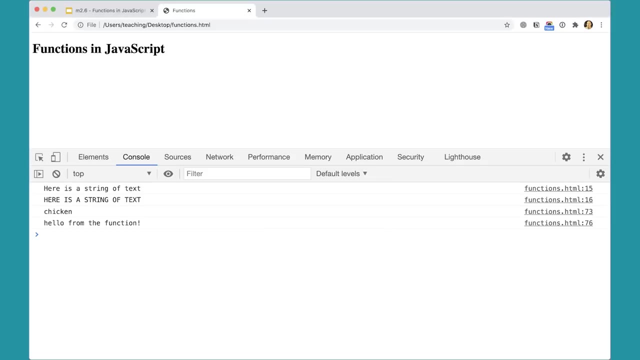 doStuff, And in that case we'll call it a function. But when a function, more explicitly, is set to work with a particular object, we're more likely to call it a method. So that's where the difference in terminology comes from. But in reality, in JavaScript, all functions are methods. 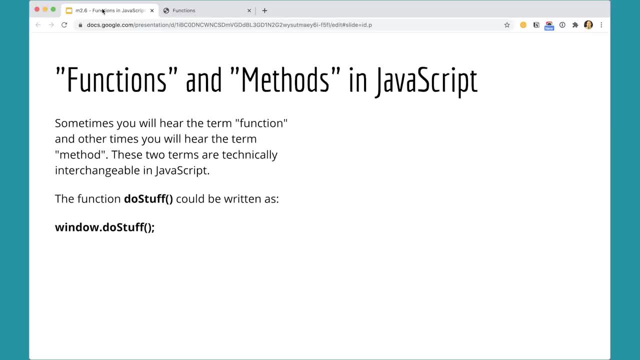 Terms really are interchangeable. So if you hear the term method and you're confused by that, just think, oh yeah, that's a function and that's fine. Okay, great, We've learned a lot about functions in this lesson and you've already learned a lot of JavaScript. And along with the challenges, 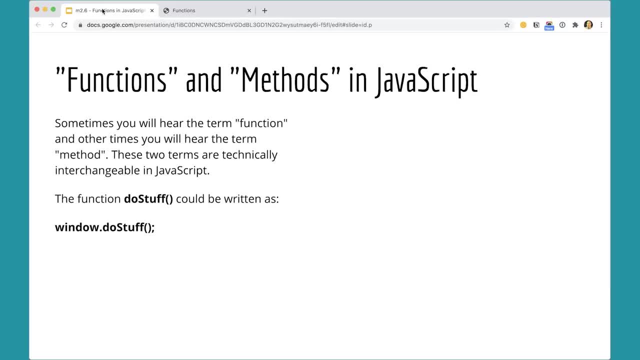 you'll really get good at the JavaScript syntax and you'll get good at being able to make simple programs function. And from here we get to start doing some much more interesting things, where we start working with content on web pages and manipulating web pages. So this course only gets more fun from here. So stick with it and keep working on the. 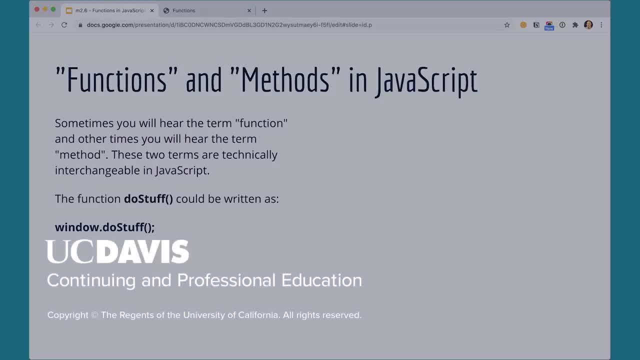 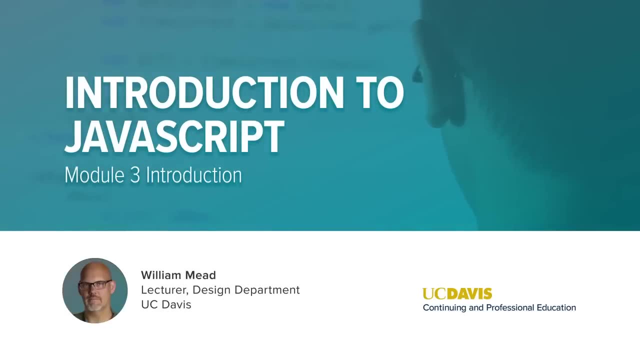 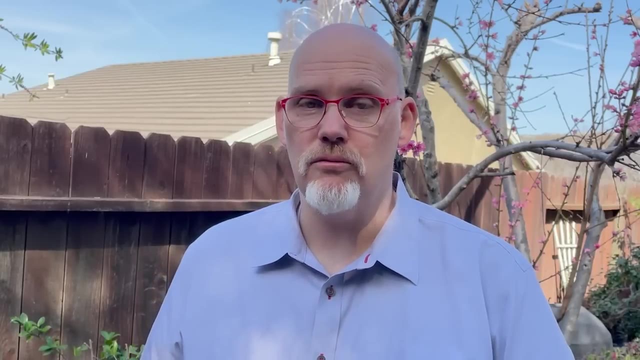 lessons and I can't wait to see you in the next one. Welcome to the third module on JavaScript. In this module we'll be doing some really exciting stuff. We'll be digging in and learning how to actually affect elements on web pages. 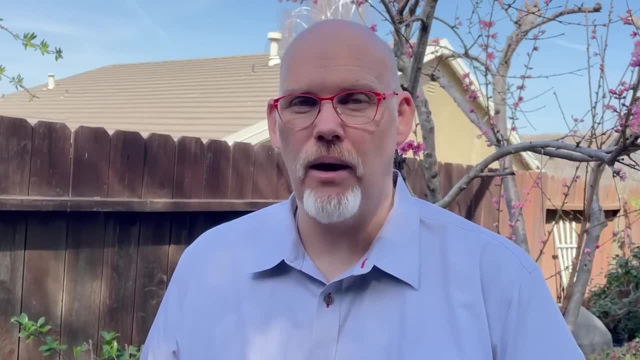 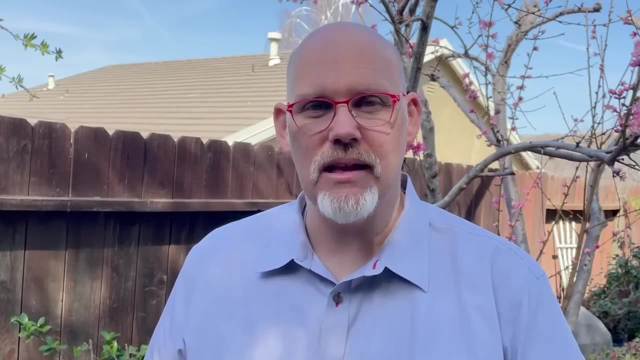 And when we do that, we'll also be looking at events. We'll look at what happens when you want to capture a click or a scroll or the submission of a form or something like that, And when we capture these events, we can then make different things happen on web pages, And this is really 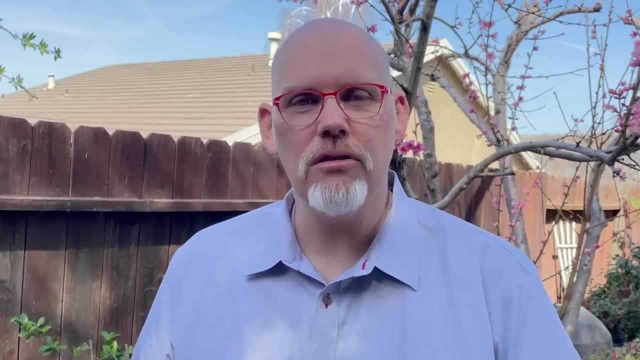 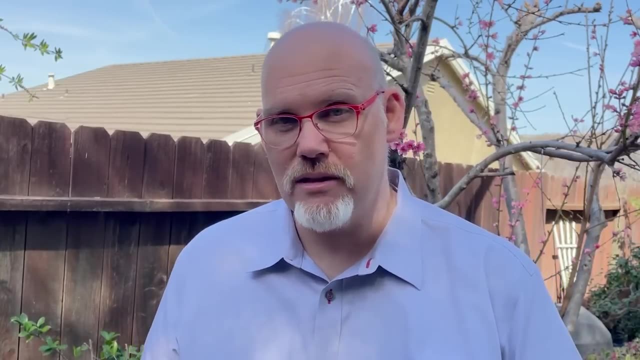 where the real magic is in JavaScript, And it's also the reason why JavaScript exists- is because it's so tightly tied. It's so tightly tied into the browser And now we can find JavaScript in other places other than the browser, but its main reason to exist is the fact that it is so tightly connected into the. 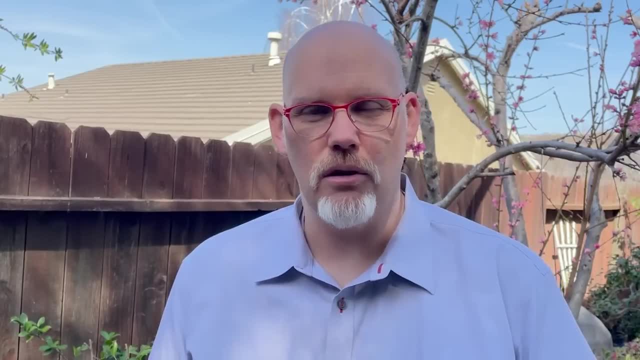 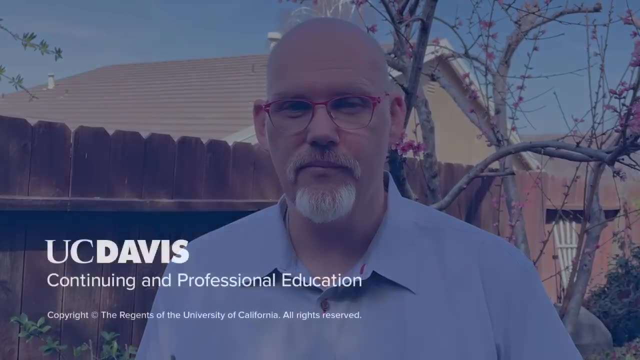 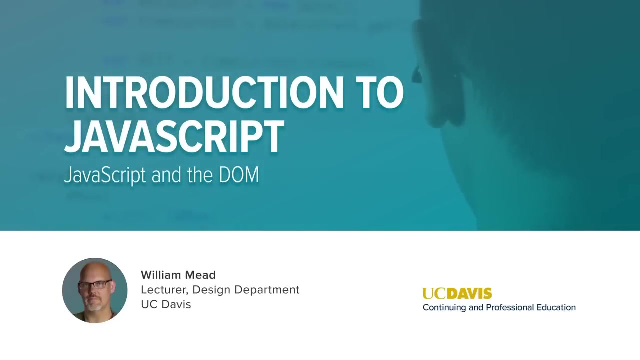 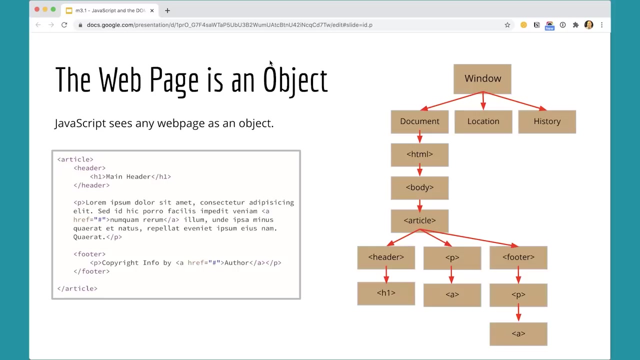 browser, And we'll really get into that in this part of this course during this module. So I hope you have fun with it And by the end you will have learned quite a lot of JavaScript, JavaScript and JavaScript, The DOM. The DOM stands for Document Object Model And JavaScript sees the web document as an object. 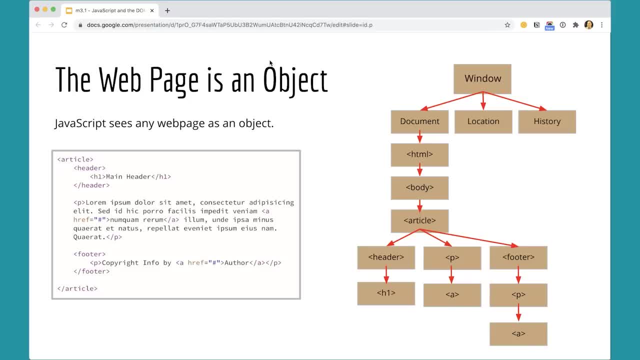 and it understands it from a hierarchical perspective. So the root object that JavaScript sees is the window itself. The window, our browser window, is the root object And then that has three sub-objects: The document, the location of that document and the history. 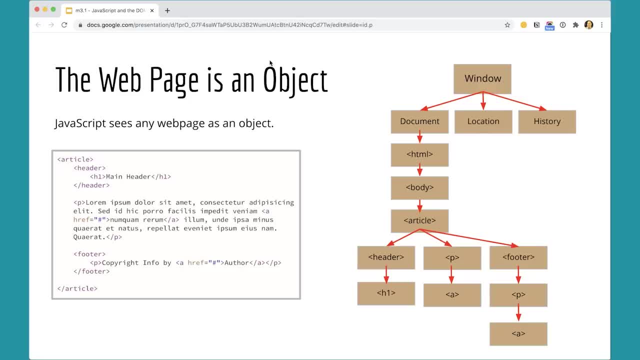 We're really concerned with the document, and the document breaks down into an HTML tag. We've seen that certainly on our documents, on our web documents, And within the HTML tag there's a body tag And then we could have whatever HTML is making up the page. Here I'm showing an article. 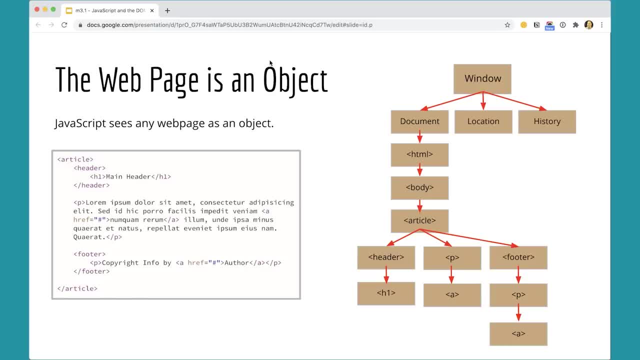 with a header and a paragraph and a footer and that matches the HTML that's in the image here on the left. so if you look at the markup on the left, you can see how that matches the article here and uh in in the diagram and uh, javascript sees the article as an object that has uh children. 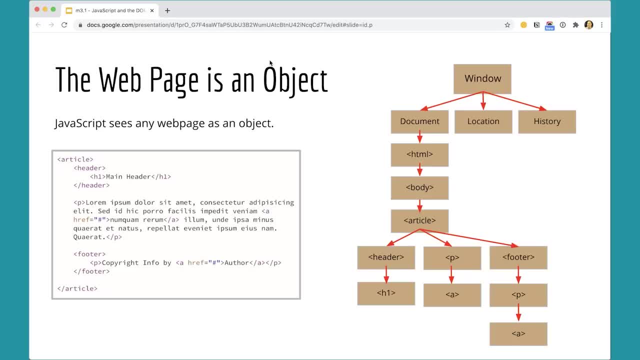 one child would be the, the header, and the header itself has a child, which would be the h1, and then another child of the article is a paragraph, and another child of the article is the footer, which also has a child which is a paragraph, and we can see that represented in 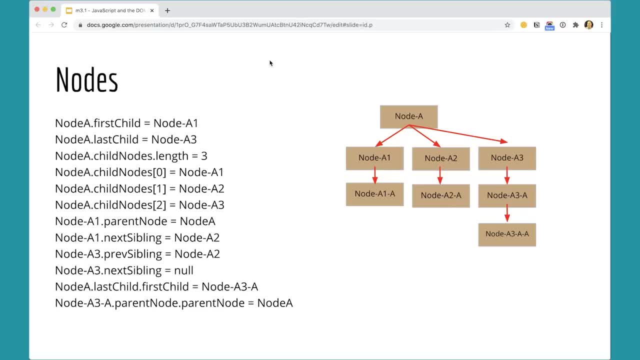 the diagram over here. these elements on the page are nodes and javascript understands the relationships between the nodes and we can use methods and properties to do what's called traversing the document and getting from one node to another so that we could affect it with javascript. so, for example, if node a was, was that article and 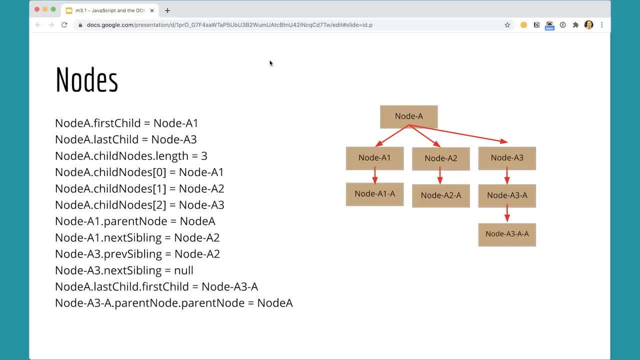 it has three children. you could say node a dot first child is node dash a1 and node a last child is node a3 and you can look through the the um, the descriptions on the left here and understand the relationships between these different elements. so node a1, dot parent node, for example, would be node a. 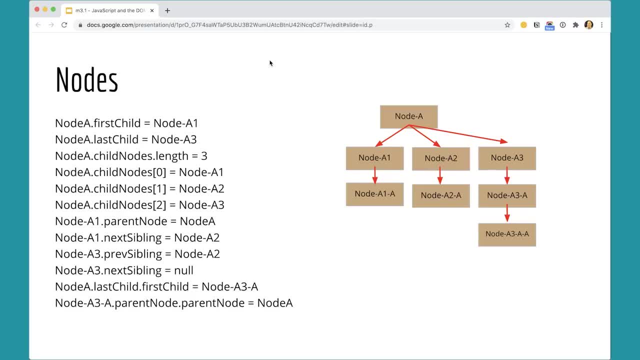 or uh, or we can look at the, the children of node a, as an array and we could say node, a child, node, square bracket zero would be node a1, and and so on and so forth, and mmm, so we could understand all the всего neighbor. 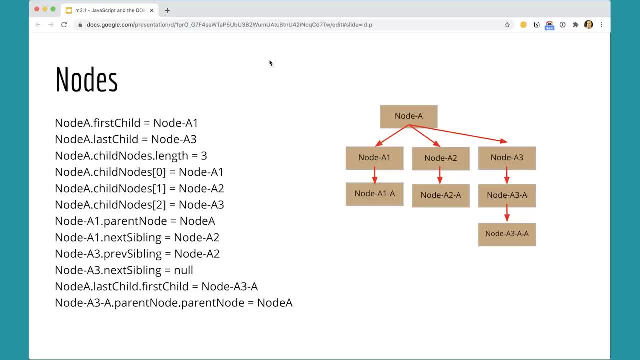 now. in other words, we also have name centro solltenrange. so this is a service that basically brings within a task a variable to a type, and then we can put it in another device and send it through. integration in with the browser and with what happens on our document is really. 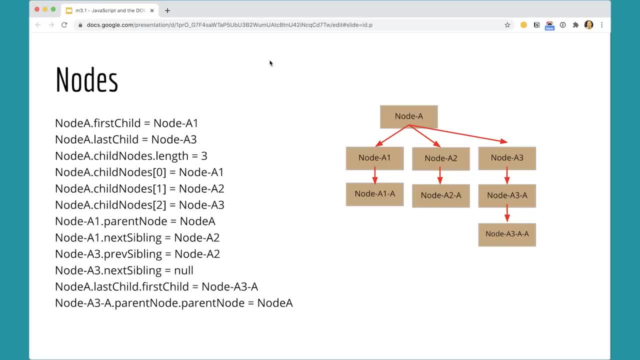 JavaScript's reason for being- and certainly we're seeing JavaScript now outside the browser and in other places- but JavaScript's main reason for being is the fact that it can do this stuff and other scripting languages can't or other programming languages can't. and in 2009, when they decided that JavaScript 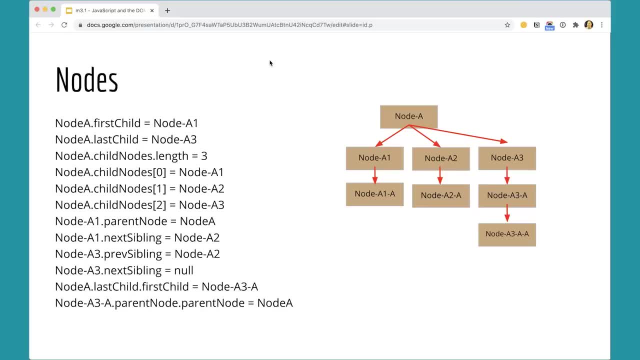 was going to be the programming language for the web. it was going to be native to the browser. that's when this stuff really got solidified and everybody wanted to follow the exact same specification and, even if they were doing slightly different implementations of it, they were following the 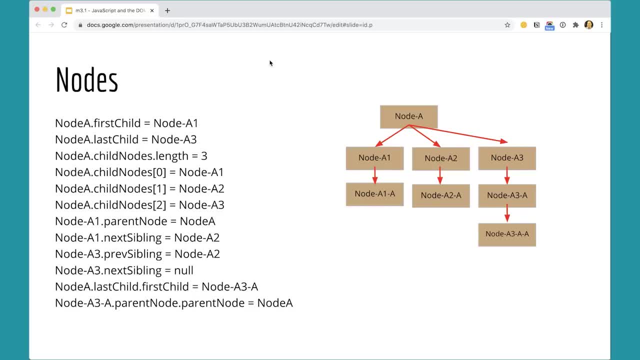 specifications that this would work with JavaScript in whichever browser you were in. it's taken a while to get to compatibility across browsers with JavaScript, but we're pretty close to there. there's a lot of things that we're going to have to do to make sure that we're 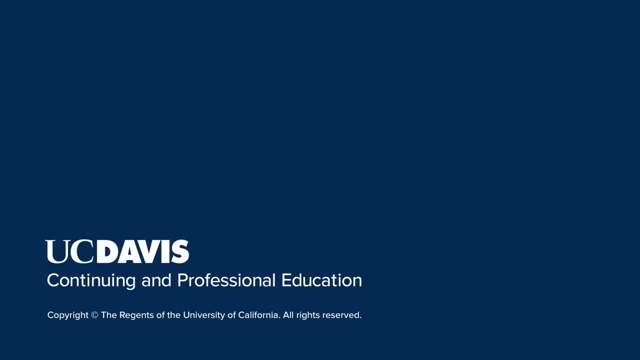 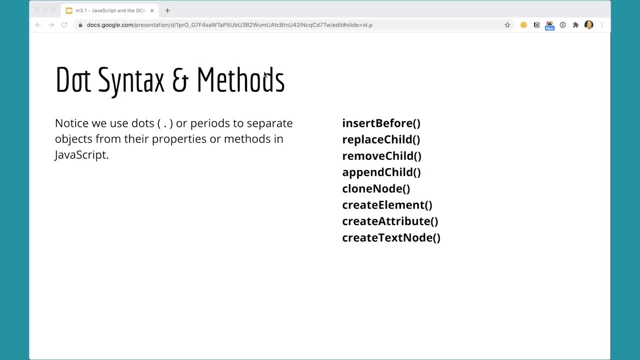 doing what we're doing these days: the dot syntax and methods notice. we use dots or periods to separate objects from their properties or their methods. in JavaScript and on the right here you can see that we have a number of methods that are related to being able to traverse the DOM or affect. 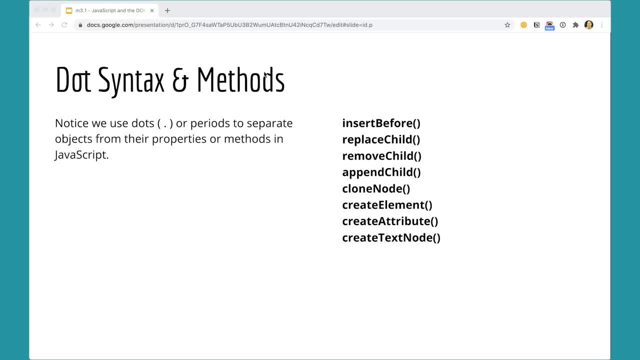 the DOM father from the way in which we we built the CSS YOURS apartment and actually, when we're inside Running we're using our abas port as an example of очень simple methods. it's called somewhere else. we can create an element, we can create attributes, we can create a text. graph. if a strong dollar and huge the form like circle data comes out before that, we're going to have to click the don't hopes object and add elements. we can also import elements to real changes that work. good for JavaScript use. answer: solid electronic block editor features. we can create an element we can insert before another element. we can replace a child. we could say: you know, take this child out of here, remove a child, append a child, append a child. we could add a new paragraph to the end of a div or something like that: clone a node. we could take an entire div with all its contents and clone it and add it to the page somewhere else. we can create an element. we can create attributes. we can create climate, A admin elements. 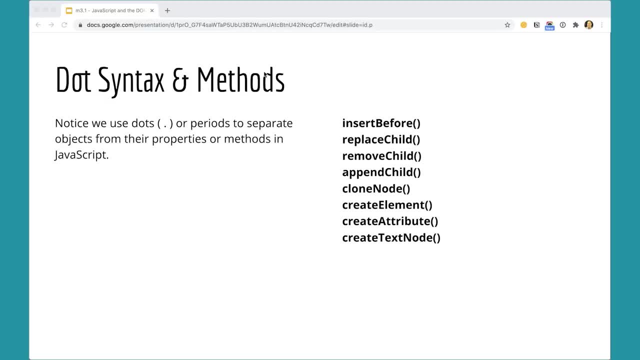 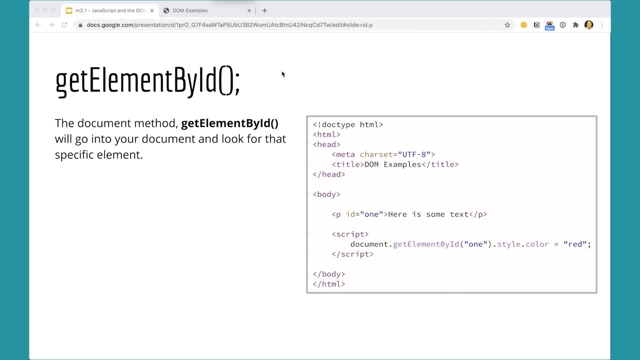 We can create a text node. These are all methods that JavaScript has built into it that allow us to do things to the document object model, to the document itself, and will affect the document there, One of the document methods you'll use most frequently. 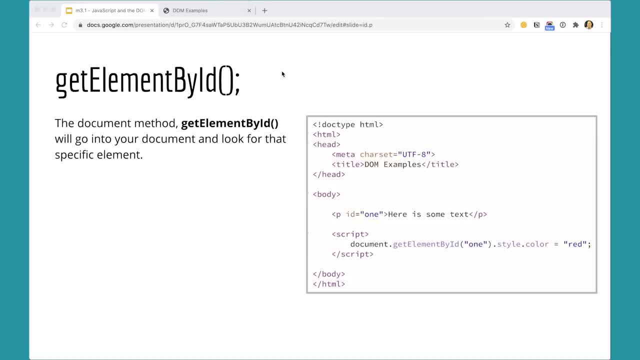 and is a good one to learn first, is getElementById. getElementById is a document, method or a function that belongs to the document object. Remember that's how we define methods, And what we can use with getElementById is we can pass in a particular ID. 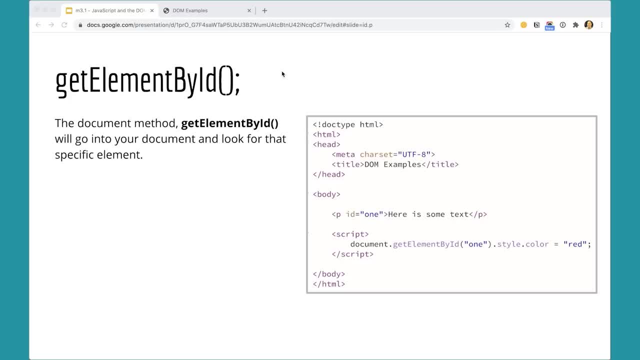 and then we can do things to that element that will go into our document, into our DOM, our document object model, and find that particular element and do something with it. So we could set the, the style property and the color sub-property to red. 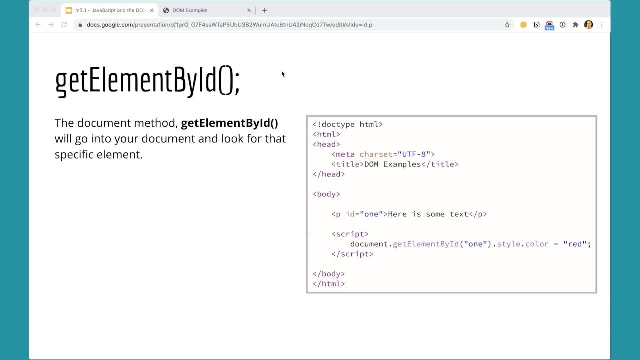 for example, for this paragraph that has an ID of one, And remember, in HTML, when you have, when you have an ID, it must be unique. It must be a unique ID on the page. This is something I see as a mistake a lot of times. 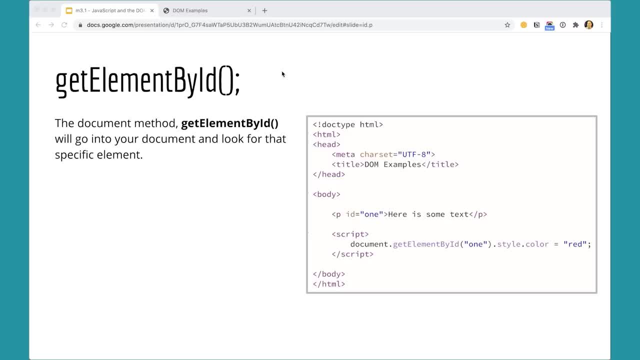 with students learning to create webpages, They'll use an ID on the page multiple times, But the whole point of an ID is that is that it's unique, Just like you have a student ID or a driver's license ID or some other ID with a unique ID number on it. 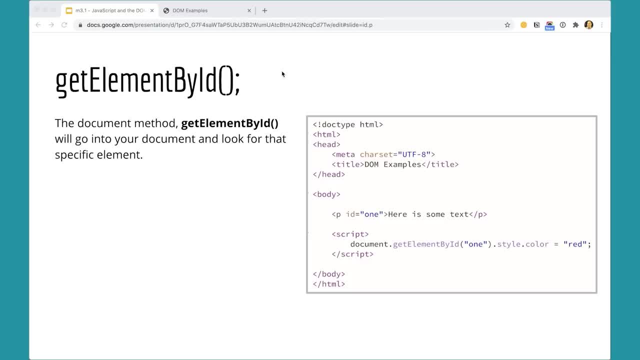 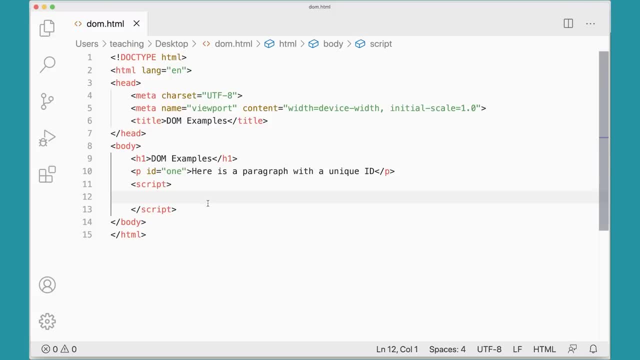 The whole purpose of having an ID is that it is unique, So let's give this a try. I'm going to come over to my code editor here and you can see I've set up a page and I guarantee it's a good idea for you to do this as well. 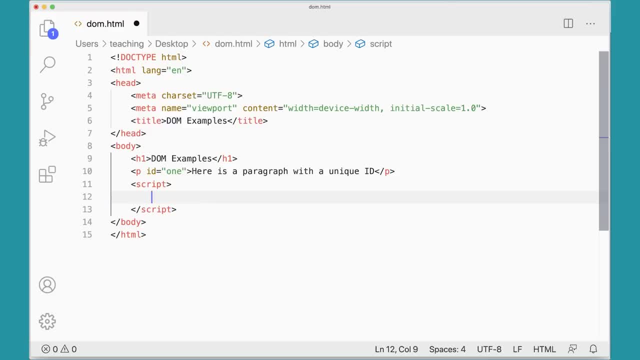 So I strongly suggest it. but I'm going to come in here and I'm going to add, I'm going to say document, If I could type documentgetElement by ID And you can see as I start typing that it even comes right up here. 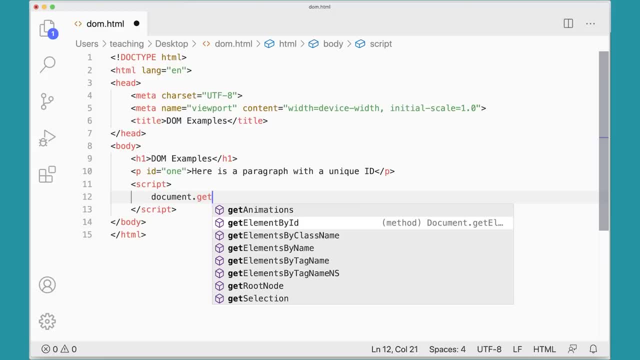 and I can actually select it from the list to make sure I get it right, Because you have to get the capitalization right. It's camel-cased, so the get is lowercase, but E is uppercase, B is uppercase and I is uppercase. 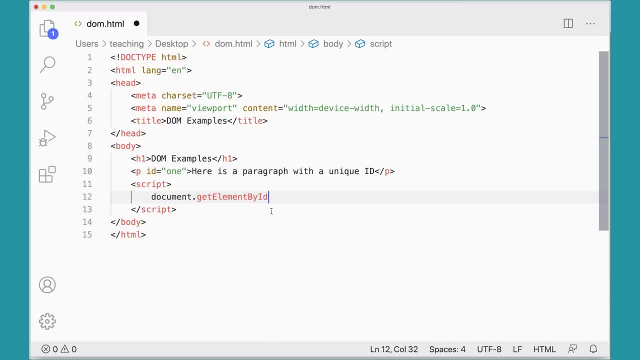 but the D is lowercase, So you have to get that right, Otherwise it won't work And I'm going to pass in 1, because it's going to match this ID here And I can set the stylecolor to red If I save that. 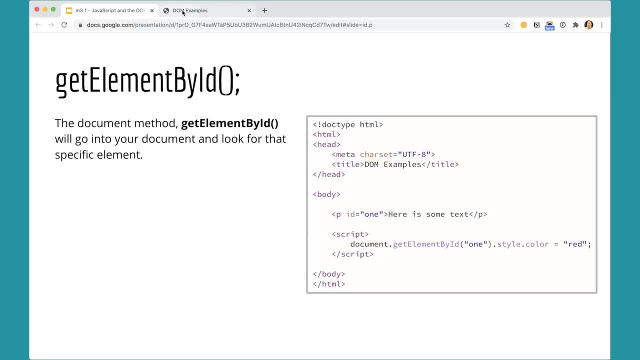 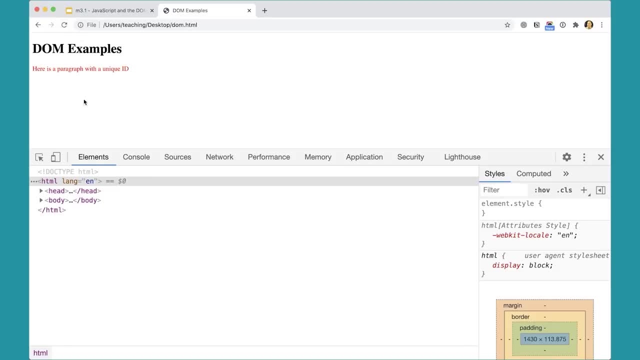 and I come back over here and you can see I have this web page loaded up here and it's black here. but as soon as I refresh the page you'll see that it's turned red. Now I don't have any code in my HTML that's doing that. 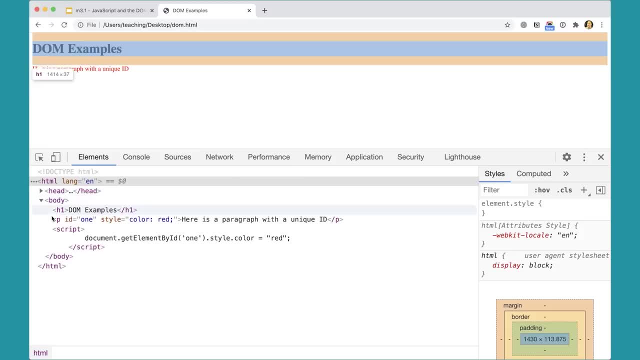 It's the script that's doing that after the fact. It's really important to understand this. So as I come down here, notice paragraph ID one and then style color red is added here, But I didn't add that. That's not in the HTML that I added. 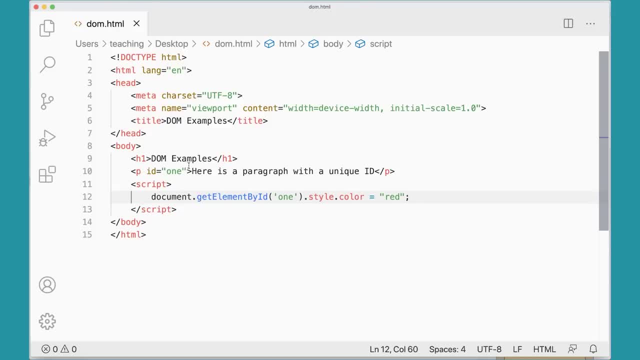 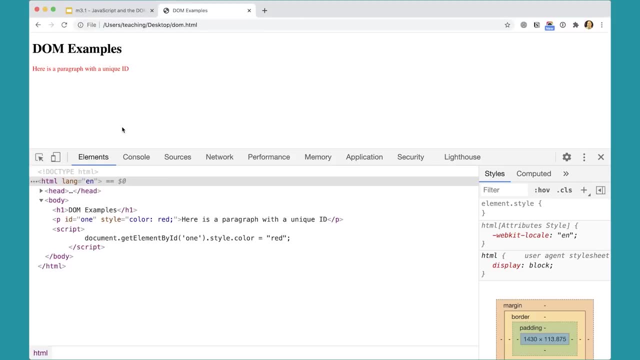 Over here in the HTML that I have. I have the ID one, but I don't have a style attribute on here at all. JavaScript took when the page loaded. JavaScript loaded the paragraph the way I wrote it, And then what the script did is: it went in and found. 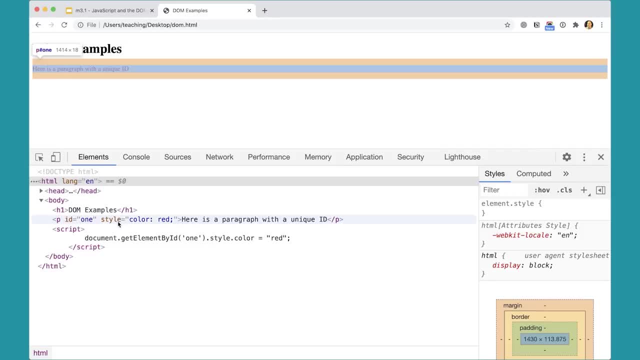 that element with the ID of one, and it added the style attribute here and set its color property to red. So JavaScript is doing that on the fly after the page has been retrieved. Right now we're just loading it from our desktop, But you could be getting it off of a web server. 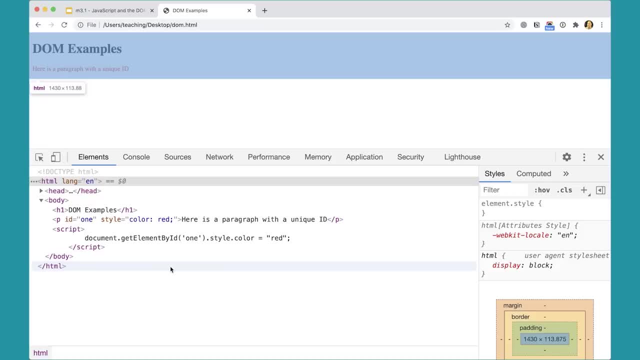 You could be getting it from anywhere And that page, when it gets to the browser, it gets rendered by the browser And then the script runs down at the bottom of the page and affects the page after that paragraph has already been rendered. It happens so fast you don't even really see it. 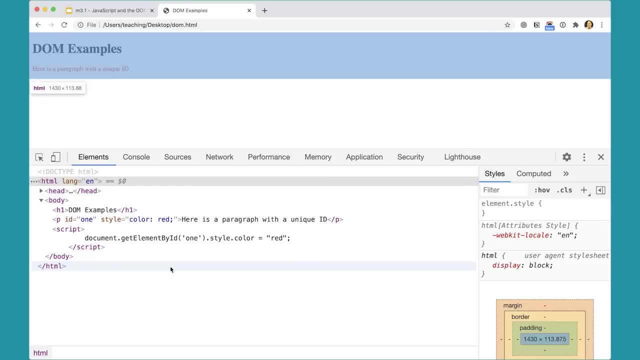 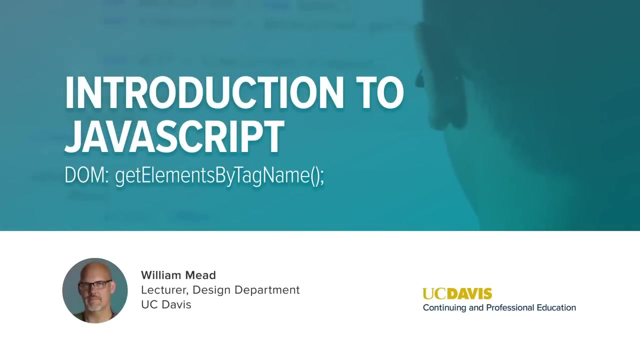 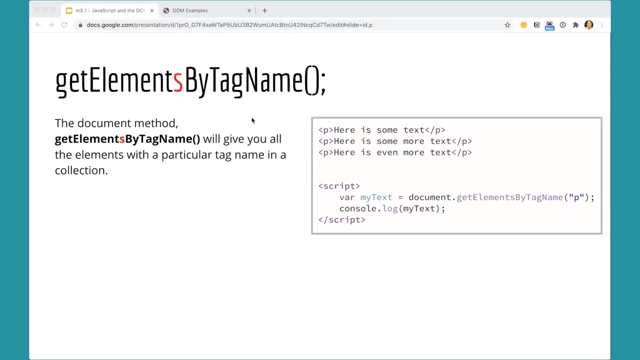 But this is a really great example of a document method- getElementById- which is allowing us to go into our document, find that ID and then affect it on the page. Here's another document method that allows us to get elements on the page. 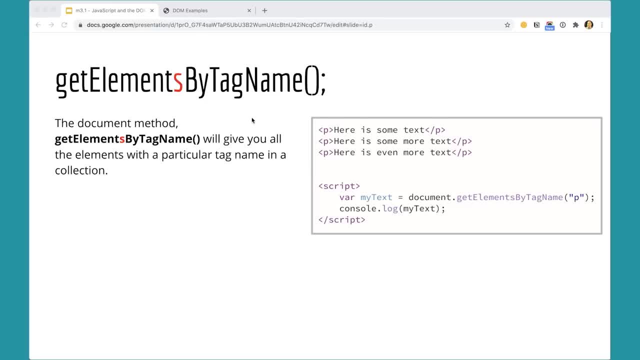 and do something with them. It's called getElementsByTagName And I have the S in elements highlighted, because a common mistake is to leave it off because it's getElementById, But this is getElements. This is going to get more than what one element is going to get a group of elements. 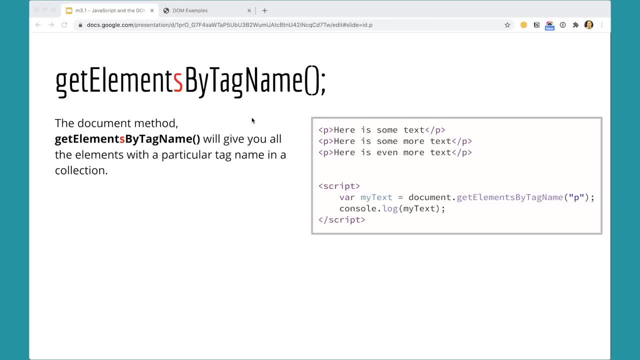 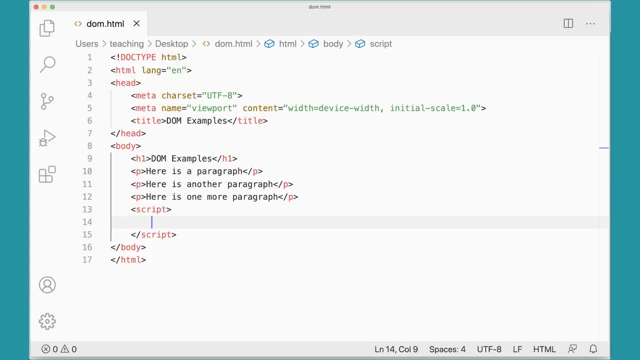 a collection of elements, And then we can do something with that collection of elements. So let's give this a try Here. I have my page, I have some paragraphs on the page And I can write a script here: documentgetElementsByTagName. getElementsByTagName. 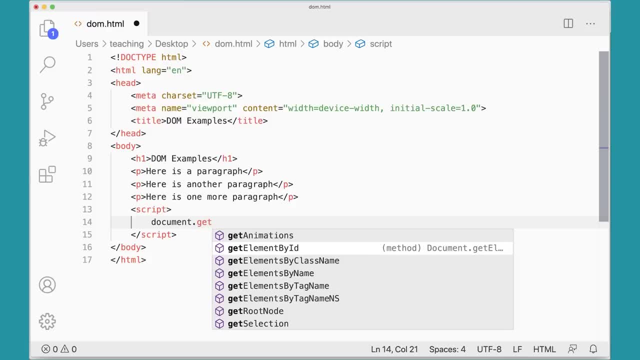 getElementsByTagName. getElementsByTagName. getElementsByTagName. getElementsByTagName. getElementsByTagName. And again, the best thing to do is to go down and make sure you select it from the list. That way you won't spell it wrong. But it's getElements with a capital E and an S by tag name. 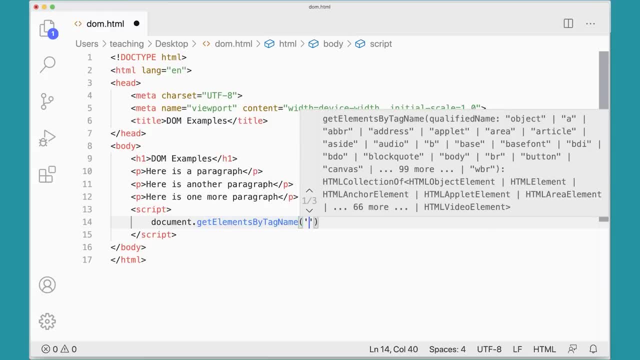 Make sure you get all the capitalization right there, And then I can actually pass in, say, a P for paragraphs. So what this is going to do is it's going to go in and get all of these elements And I can assign that to a variable. 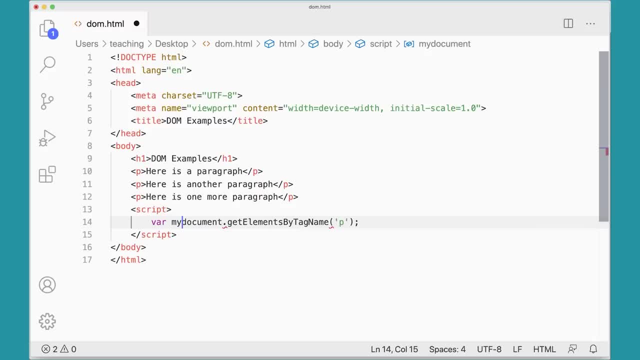 getElementsByTagName. getElementsByTagName var. myParagraphs equals. So now myParagraphs is going to hold a collection of paragraphs And if I consolelog that out, consolelog myParagraphs. if I consolelog that out, let's see what I get. 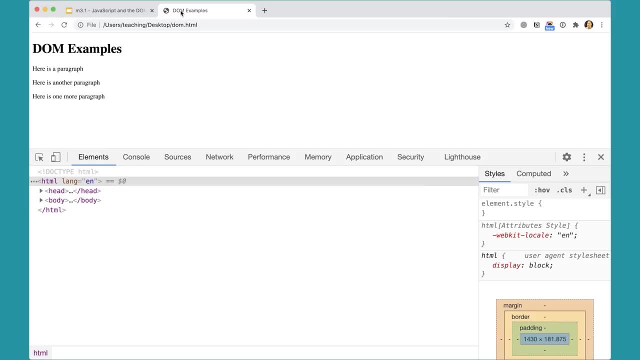 I'm going to come back over here to my page and refresh And we don't see any difference here. But if I go to the console, you'll see I get an HTML collection of three things: paragraph, paragraph and paragraph, And that's what's in here. 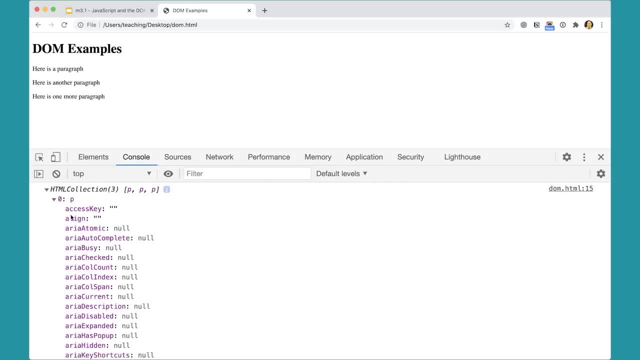 And I can even fold this down and see what the different paragraphs are. It gives me some information about them, But it's giving me the collection of the paragraphs here, So that's kind of important to understand about this particular method, Whereas getElementById gives me always just one thing. 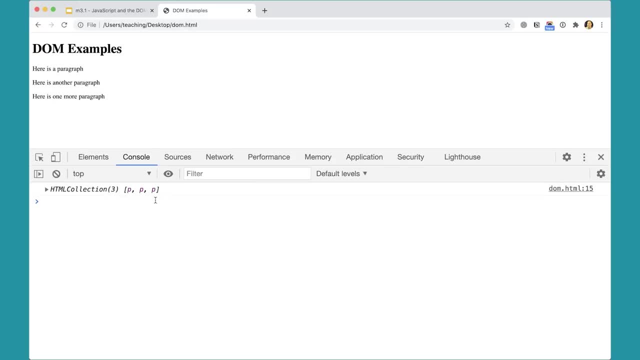 It'll always give me one, because id's are unique, Whereas getElementsByTagName will give me an HTML collection of elements that I need to then do something else with. If I wanted to set the color of these paragraphs, I could do that getElementById. 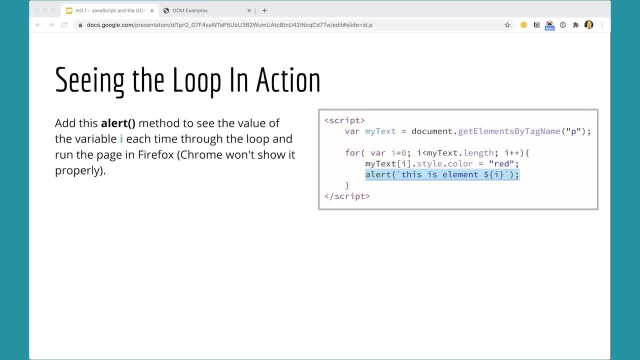 getElementById, getElementById, getElementById, getElementById to red, then I would need to use a loop, because I can't apply the style color to a collection of things all at once. I have to apply them to each item in that collection, So I need to use a loop. 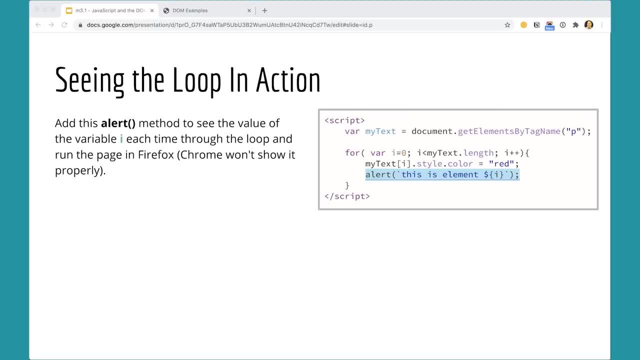 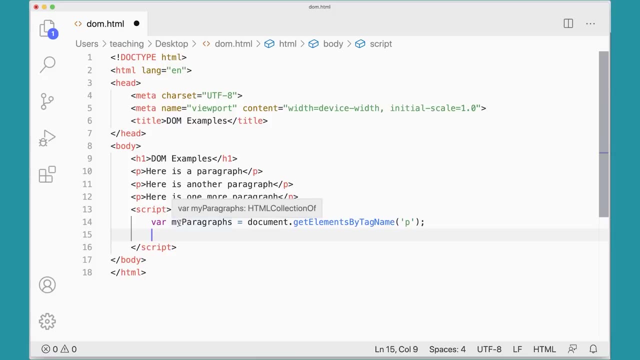 to loop through each of the elements in that collection. So I'm going to use a for loop here And let's go ahead and do this over here Rather than console log this out. I'm going to use a shorter variable here. My paragraphs is kind of long, I'm guaranteed to. 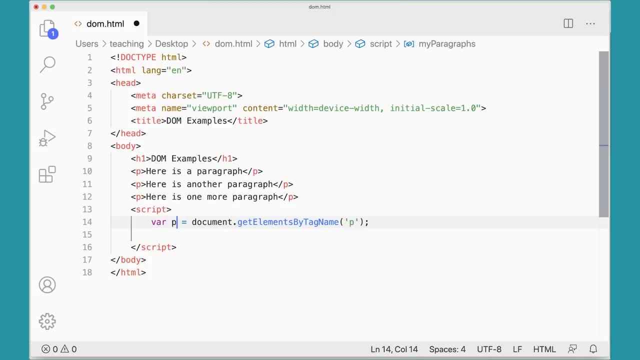 type that wrong at some point, So I'm just going to call it peas, something like that. That's fine for paragraphs. That's fine, All right, great. So I'm going to make a for loop And again remember if you've been doing the challenges and really getting used to the syntax. 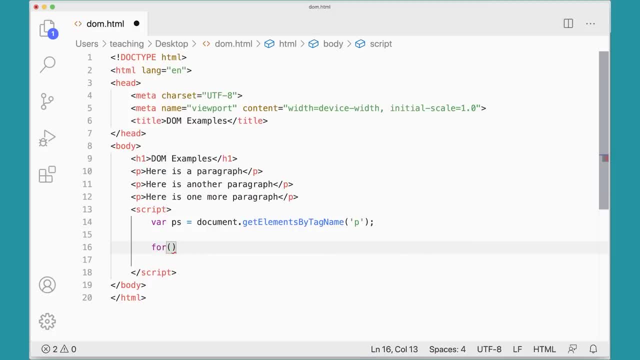 you should be able to just write a for loop For var i equals 0,, while i is less than peaslength i++. And then we've got our curly braces And in here I'm going to take each paragraph. So I'm going to say: peas, square bracket i dot. style dot color equals red. 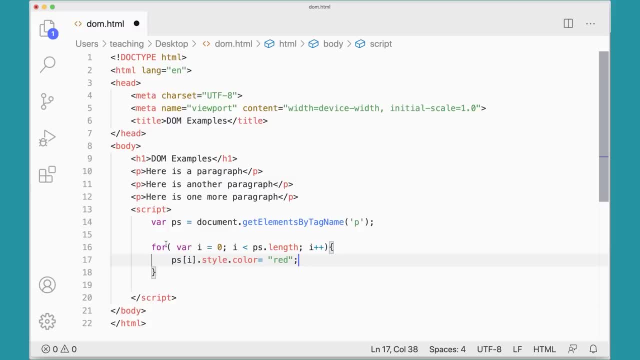 Now, if I just do this, you'll see it'll work. It'll actually go through this entire loop The first time through the loop. this thing has three paragraphs And it's going to get paragraph 0 and set its style color to red, And then i gets incremented from 0 to 1.. 1 is less than 3.. 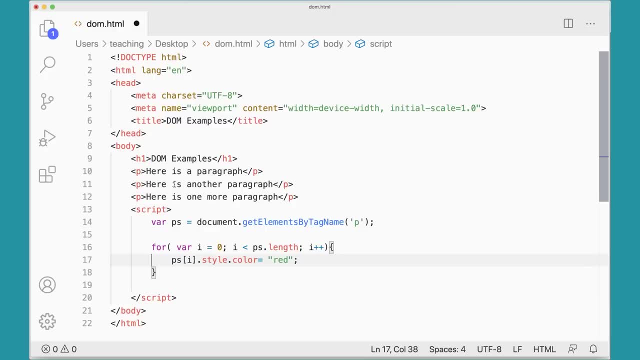 So it will get paragraph 1, which is this one here, and set its color to red. i gets incremented again to 2.. 2 is less than 3. So it'll come in. It'll get paragraph 2, this one here, and set its color to red. 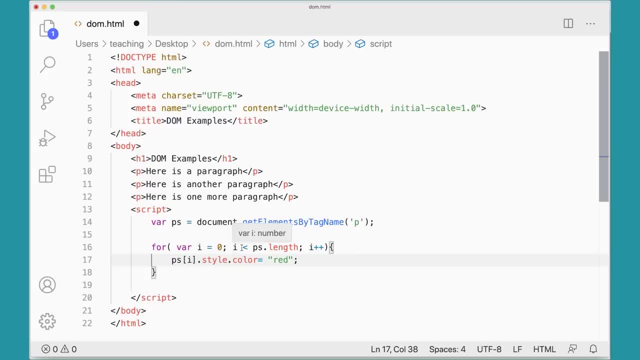 And then i gets incremented to 3.. 3 is no longer less than 3. Because remember peas dot length, the length of this is 3.. So 3 is no longer less than 3 in the script. So let's give that a try. Let's run that over here. 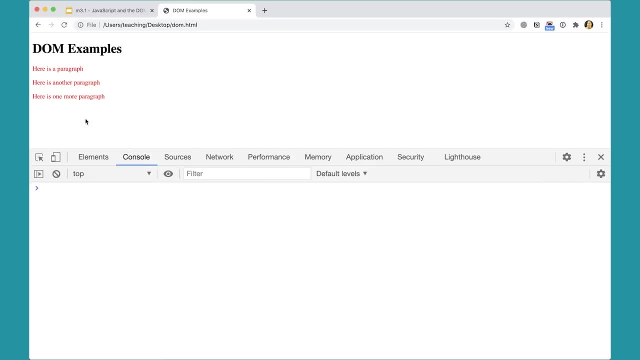 If I refresh this, you can see all my paragraphs turn red. Now the loop goes so fast You can't even see it, So let's do something to make it so we can really see that this is actually. I think this is kind of interesting. 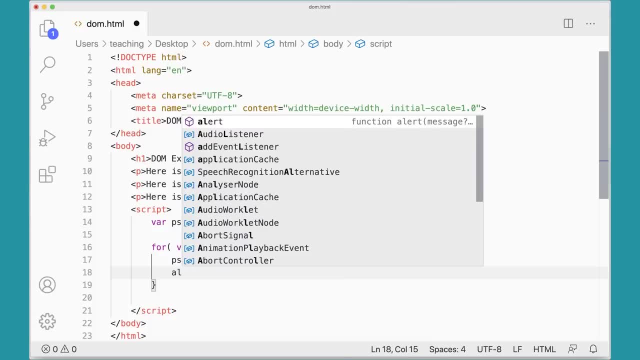 I'm going to come in here and I'm going to add alert. I'm going to use my back ticks here, Showing paragraph I. And then, don't forget, since that's going to be a variable, we're going to dollar sign: curly brace, curly brace. 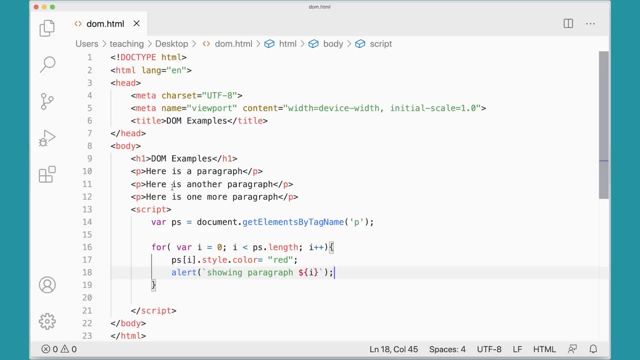 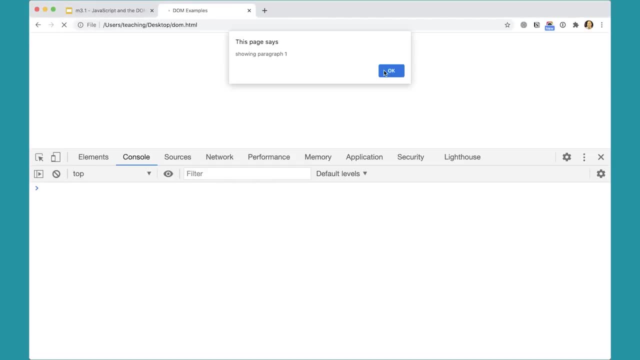 Now, if I run this in Chrome, I'm going to get this alert three times: Showing paragraph zero, showing paragraph one, showing paragraph two, and then it turns the colors. Even better is to show this in Firefox, So I'm going to switch to Firefox web browser over here. 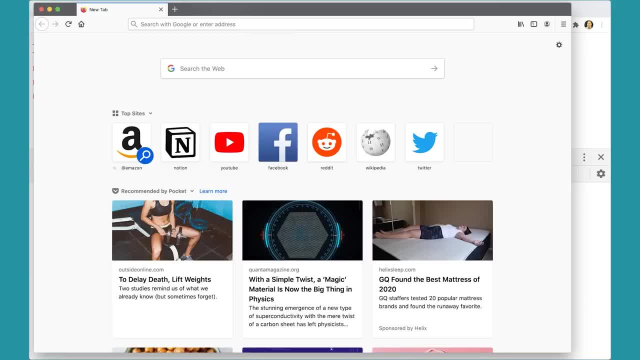 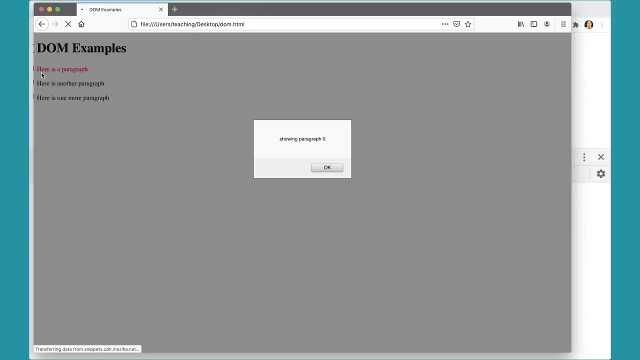 Firefox does things a little bit differently. It uses the Mozilla rendering engine, And so it renders things a little bit differently. So I'm going to go ahead and open our page here in Firefox- And there's my- And notice the difference here. 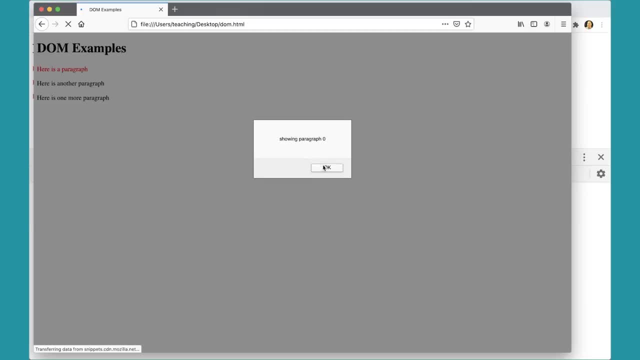 This one actually shows the first paragraph turns red And then I get the alert, And then we see the second paragraph turn red And I get the alert, And then I get the third paragraph turning red, So you can actually see the loop actually running. 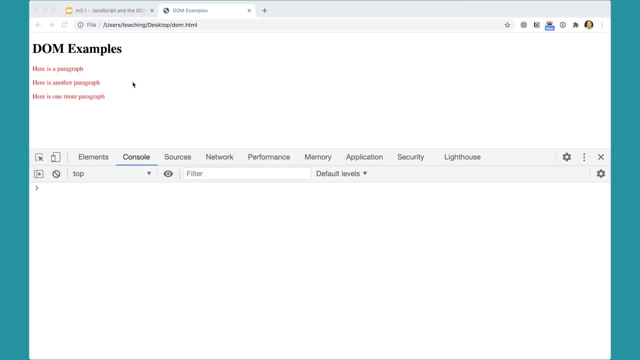 And usually these loops run so fast you don't even see them. But with the alert in there you can actually see that that loop is running And turning the paragraphs red, one at a time And then the other one at a time in the collection. 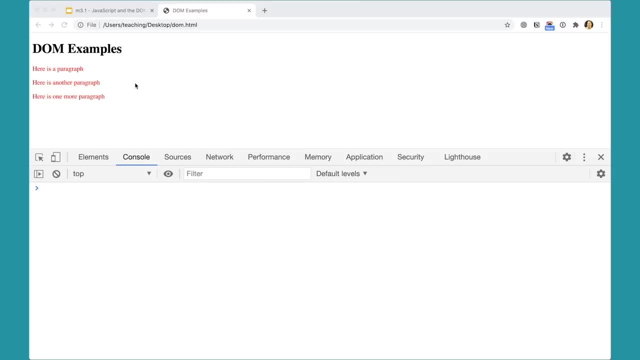 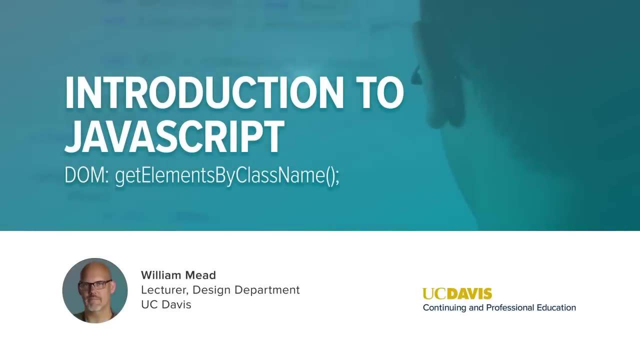 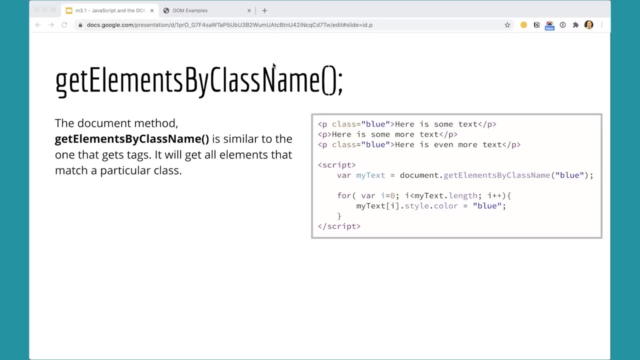 And I think that that's helpful in understanding how JavaScript works with collections of elements. The next document method that we're going to look at is getElementsByClassName, And this method will do exactly what you think it will do. It will allow us to go into our document and get elements that have a particular class name. 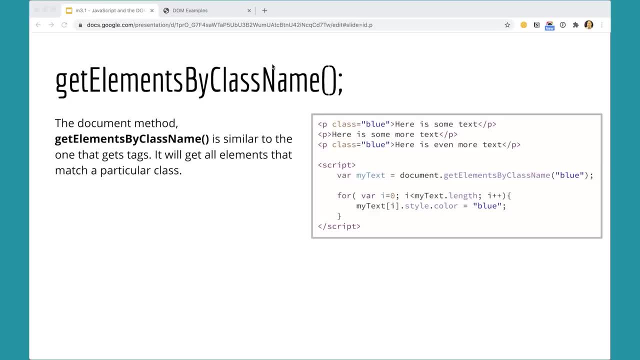 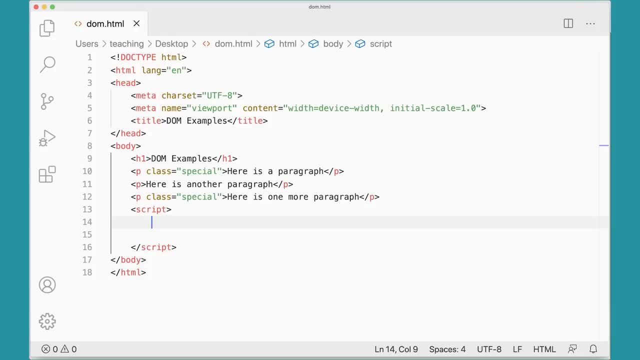 And it will tell us what class it is, class name and put them into an HTML collection. so that's very useful as well. let's give it a try real quick. here you can see I've added class equals special. on my image over there was blue, but whatever, whatever class you want to. 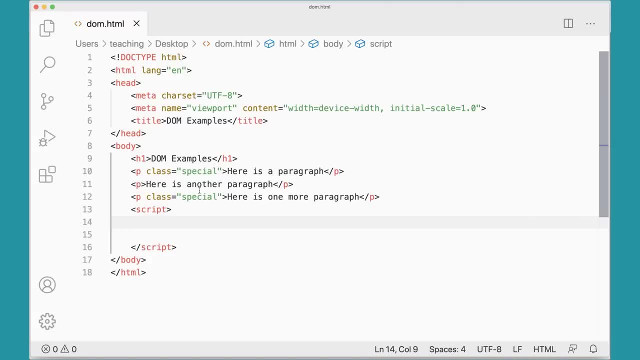 put is fine. it doesn't really matter as long as you set up a variable bar. my class equals document dot. get elements by class name. this one here and again. make sure you get all the capitalization right or it won't work and we're gonna get special. make sure you spell the same as it is there and I'm likely to spell. 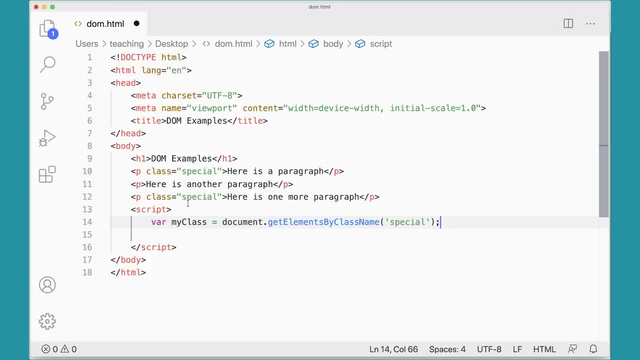 that wrong. so that will take all of these elements- in this case it's just two- and stick them to a into a collection and then, the same as before, we're going to need to use our, use our loop to go through and change these items or bar. I. 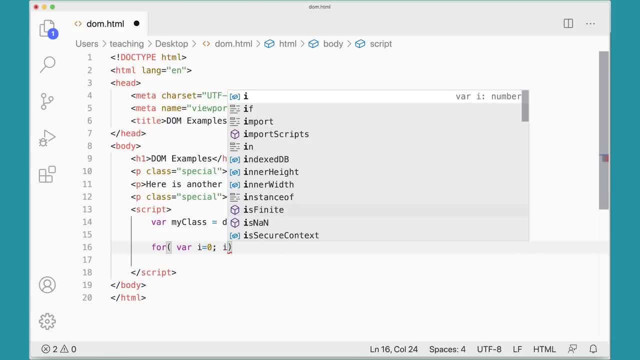 equals zero. well, I is less than my class dot length. I could just prove it, but I don't think it's going to work. I could just prove it, but I don't. I could just prove it, but I don't think it's going to work. I could just prove. 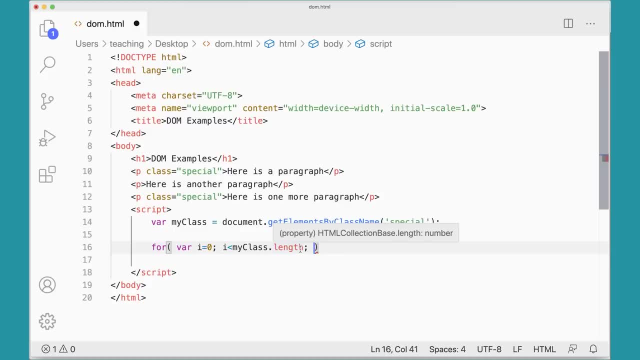 it, but I don't think it's going to work. I could just prove it, but I don't think it's going to work. put a two there, but it's better to use this just to make sure that I get all of. put a two there, but it's better to use this just to make sure that I get all of. 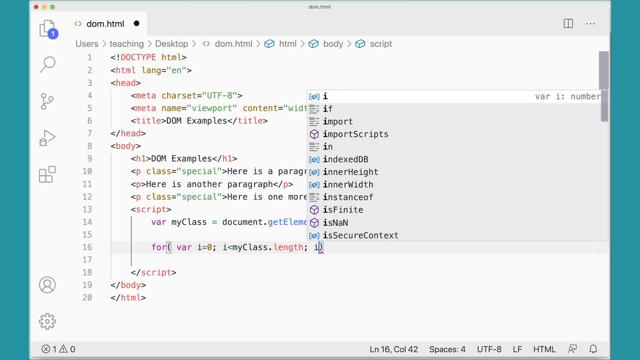 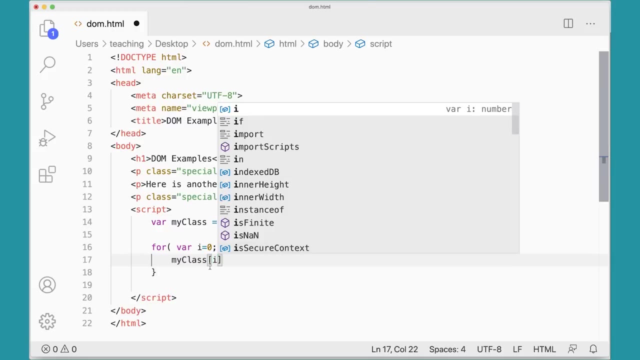 them, no matter how many there are all right plus plus, and then I could do my them. no matter how many there are all right plus plus, and then I could do my them. no matter how many there are all right plus plus, and then I could do my class square bracket. fine, first time to the class square bracket- fine, first time to the class square bracket- fine, first time to the loop. that's going to be a zero second loop. that's going to be a zero second loop. that's going to be a zero. second time to the loop. it's going to be a one. 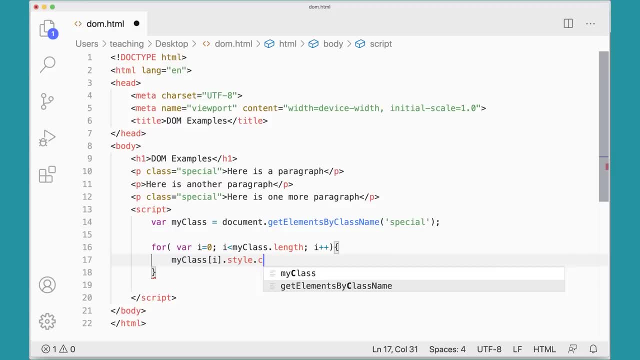 time to the loop. it's going to be a one time to the loop. it's going to be a one, and then it'll finish dot style, dot color, and then it'll finish dot style, dot color, and then it'll finish dot style, dot color equals red, and that should work just. 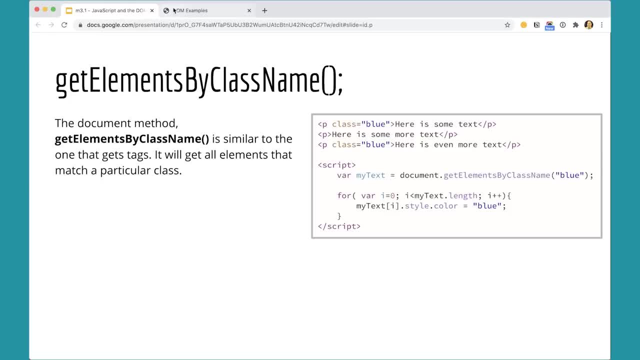 equals red, and that should work. just equals red, and that should work, just fine. let's go test it out and it turned fine. let's go test it out and it turned fine. let's go test it out and it turned. those two classes. right now one more. 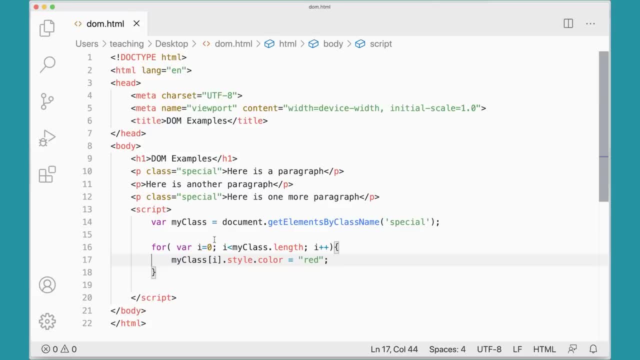 those two classes right now. one more: those two classes right now. one more point of interest while we're here, even point of interest while we're here, even point of interest while we're here, even if I just had one element on the page, if I just had one element on the page. 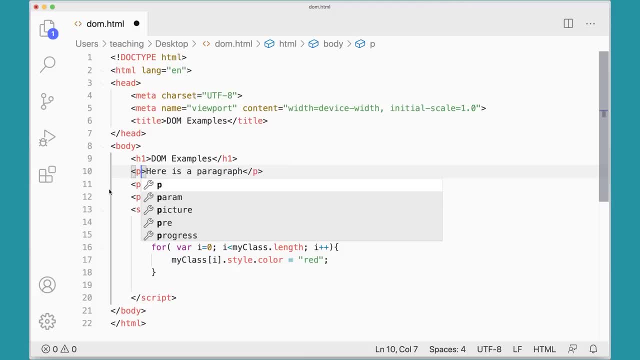 if I just had one element on the page that had this class, that had this class, that had this class, I could give it an ID and use get element. I could give it an ID and use get element. I could give it an ID and use get element by ID. but if I am going to use get, 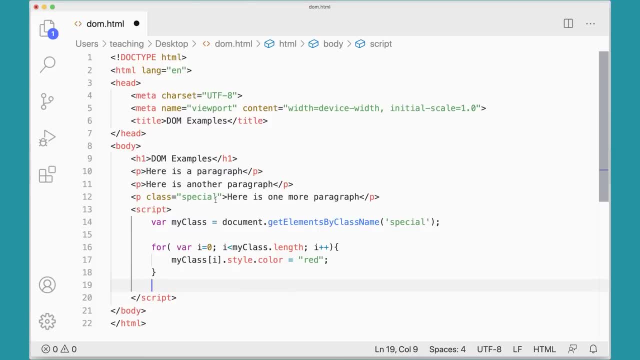 by ID, but if I am going to use get by ID, but if I am going to use get elements by class name, even if there's elements by class name, even if there's elements by class name, even if there's only one, it still is going to return a. 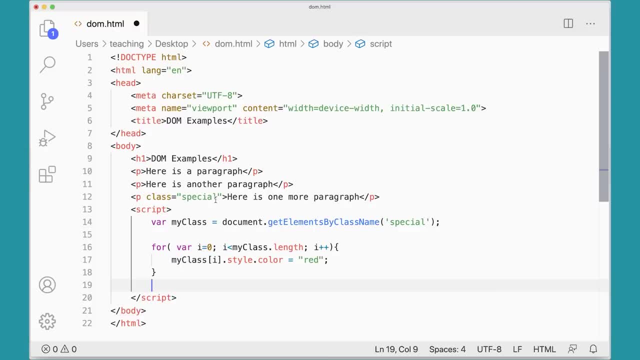 only one. it still is going to return a only one. it still is going to return a collection of elements and that collection of elements and that collection of elements and that collection is only going to have one collection is only going to have one collection is only going to have one element in it, and I still need to use a. 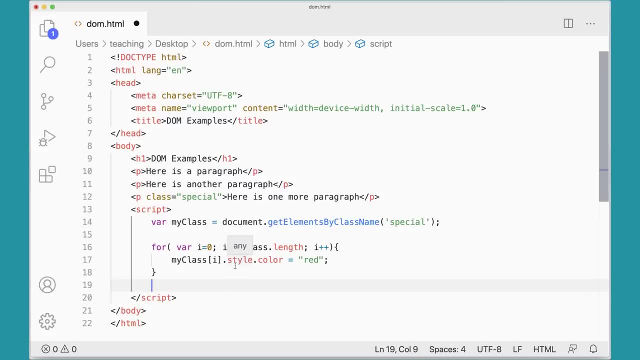 element in it and I still need to use a element in it and I still need to use a loop or some other way of getting to loop, or some other way of getting to loop, or some other way of getting to the element inside the collection, even the element inside the collection, even. 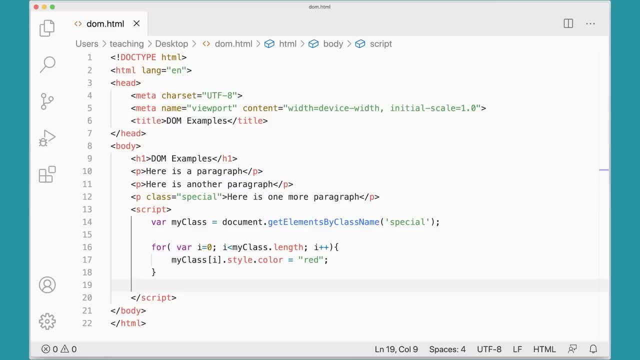 the element inside the collection, even though there's only one, and you'll see, though there's only one, and you'll see, though there's only one, and you'll see, the loop will still work, it'll just run. the loop will still work, it'll just run. 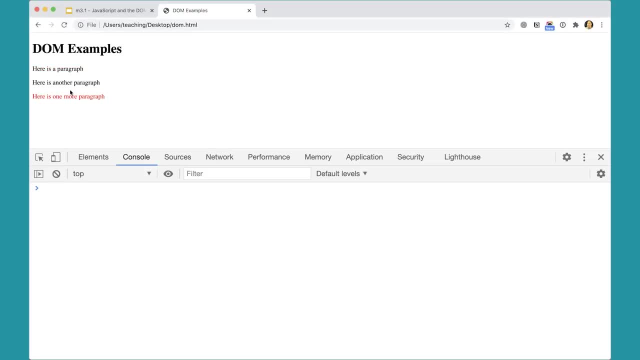 the loop will still work. it'll just run only one time. a little bit easier way of only one time. a little bit easier way of only one time. a little bit easier way of doing this. I don't really need a loop doing this. I don't really need a loop. 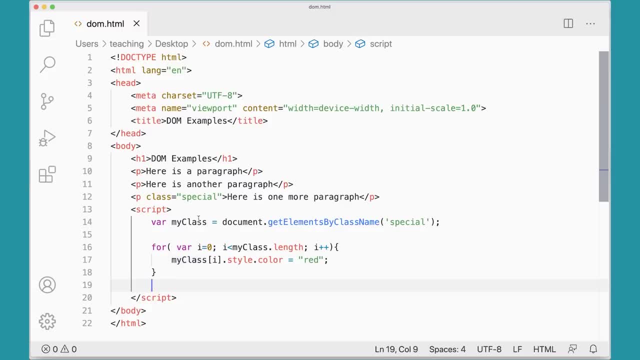 doing this. I don't really need a loop here, because I know that it's only good here. because I know that it's only good here, because I know that it's only good, there's only one element in this. there's only one element in this. there's only one element in this collection. so I know it's gonna be on. 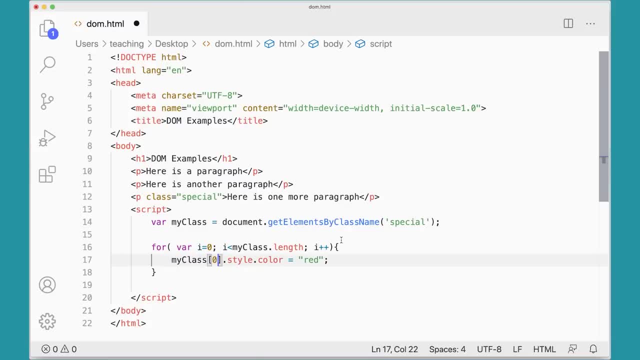 collection, so I know it's gonna be on collection, so I know it's gonna be on zero, so I don't need a loop. I can just zero, so I don't need a loop. I can just zero, so I don't need a loop. I can just make this zero, get rid of the loop, like. 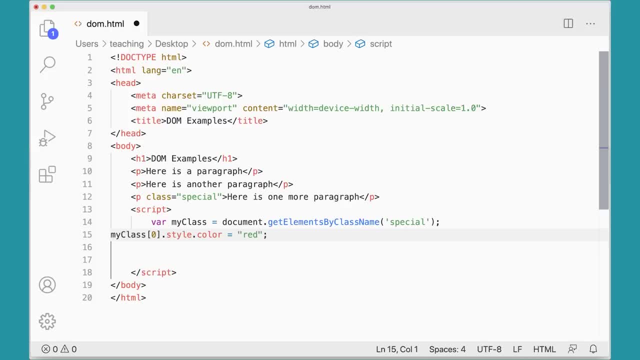 make this zero get rid of the loop. like make this zero get rid of the loop. like so kind of clean that up a little bit. so kind of clean that up a little bit, so kind of clean that up a little bit. so now I've got, my class is getting. 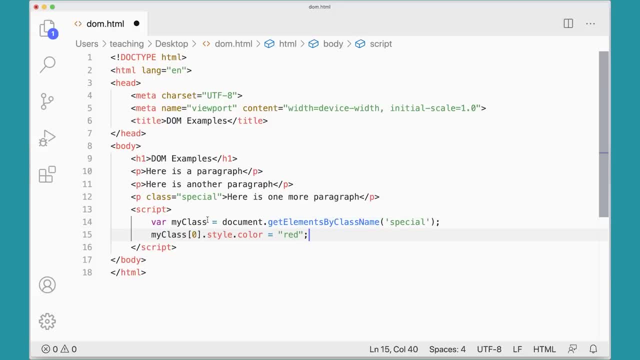 now I've got my class is getting. now I've got my class is getting- elements by class name special and my elements by class name special and my elements by class name special and my class 0, since I know there's only one class 0, since I know there's only one. 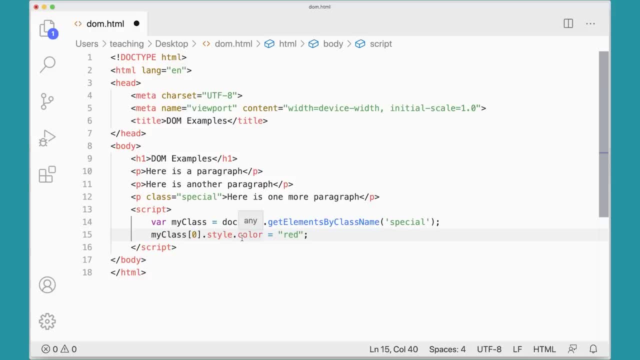 class 0, since I know there's only one. it's gonna be my class 0. it's gonna be. it's gonna be my class 0, it's gonna be. it's gonna be my class 0. it's gonna be that one in in the collection, so I can. 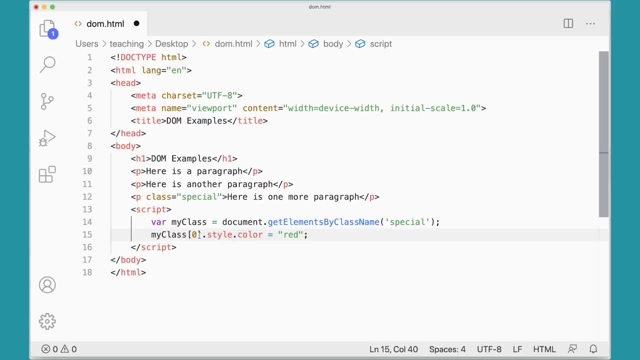 that one in in the collection so I can that one in in the collection so I can access it through because it's it's access it through, because it's it's access it through, because it's it's treated like an array there. it's not treated like an array there, it's not. 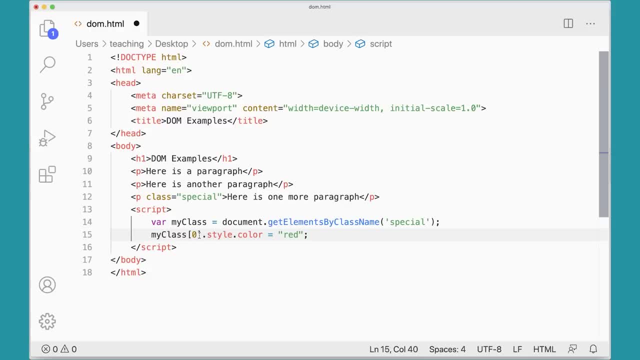 treated like an array there. it's not actually an array. it's a collection of actually an array. it's a collection of actually an array. it's a collection of HTML elements but I can treat it like an HTML elements. but I can treat it like an HTML elements but I can treat it like an array to go and get element 0 out of. 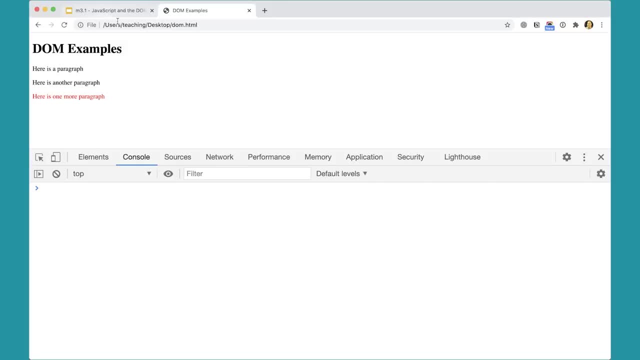 array to go and get element 0 out of array. to go and get element 0 out of there, and you'll see that will work just there and you'll see that will work just there and you'll see that will work just as well. but the important thing here to 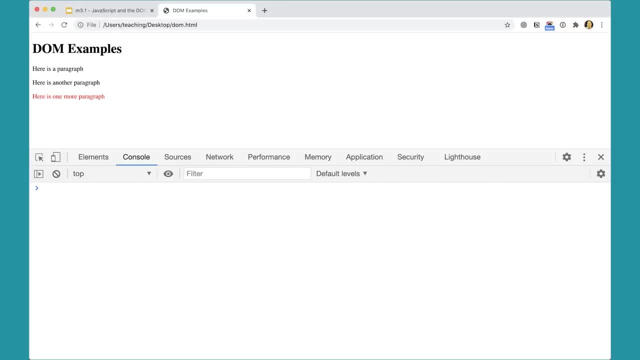 as well. but the important thing here to as well. but the important thing here to understand is that if you're using get understand is that if you're using get understand is that if you're using get elements by class name or get elements, elements by class name or get elements. 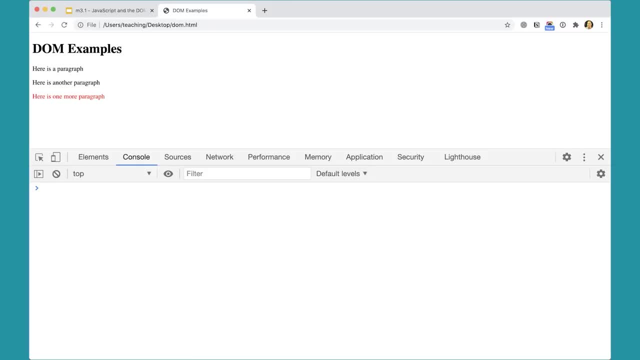 elements by class name or get elements by tag name or anything else that gives by tag name or anything else that gives by tag name or anything else that gives you a collection of elements. you have to you a collection of elements. you have to you a collection of elements you have to. you have to go in and treat it as it's. 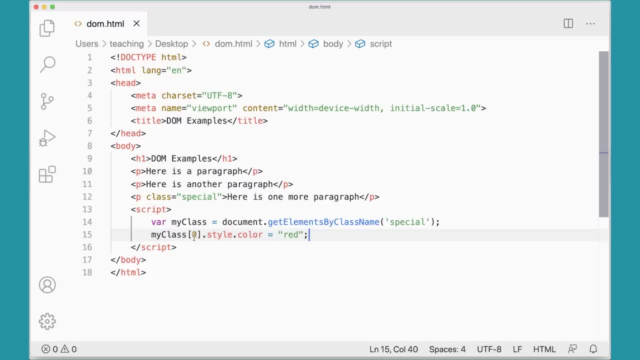 you have to, you have to go in and treat it as it's, as if it's a collection, as if it's a collection, as if it's a collection because that's what it is, and not just because that's what it is, and not just because that's what it is and not just as an individual element, and that's easy. as an individual element, and that's easy as an individual element, and that's easy to forget, especially if you have only to forget, especially if you have only to forget, especially if you have only one. you're like: how come I can't just one? you're like: how come I can't just 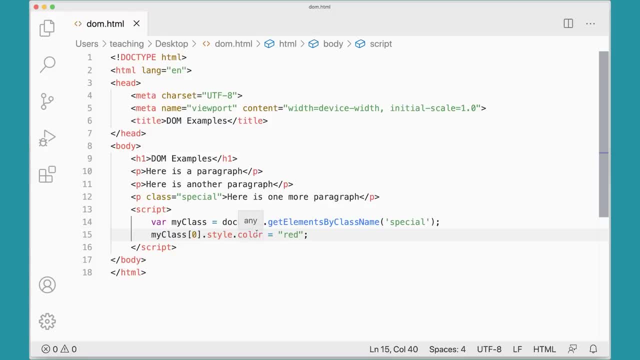 one. you're like: how come I can't just change that one? you know why can't I change that one? you know why can't I change that one? you know why can't I just use my class style color red? just use my class style color red. 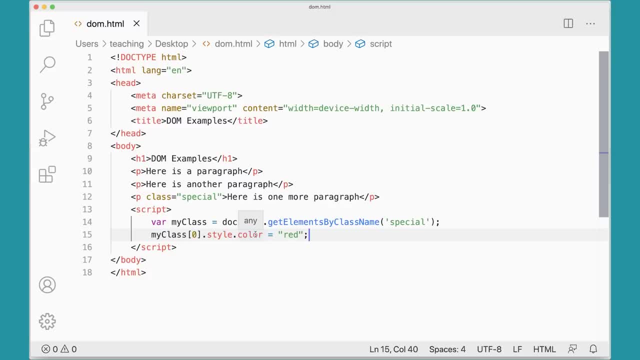 just use my class style color red, because there's only one element with that class in there. but javascript is getting a collection of elements. even if the collection only has one element, or even if it has zero elements, it'll still be a collection of elements. so that's an important thing to understand about get elements by class name and get elements by tag. 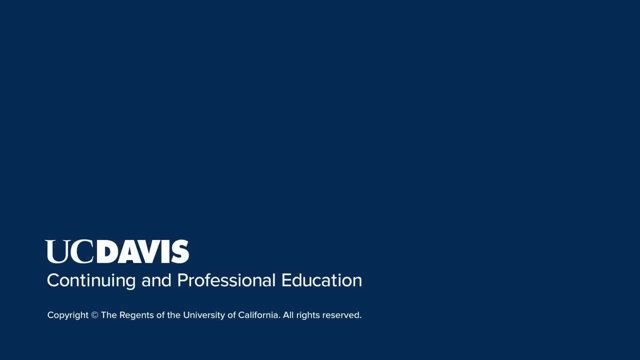 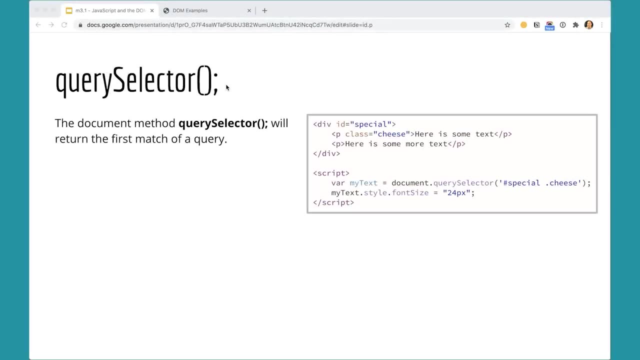 name. the next document method that we're going to look at is is query selector. now, the history here is a little bit interesting because in 2009, as we said before, es5 became the de facto standard for scripting for the web, but there was the rise of a. 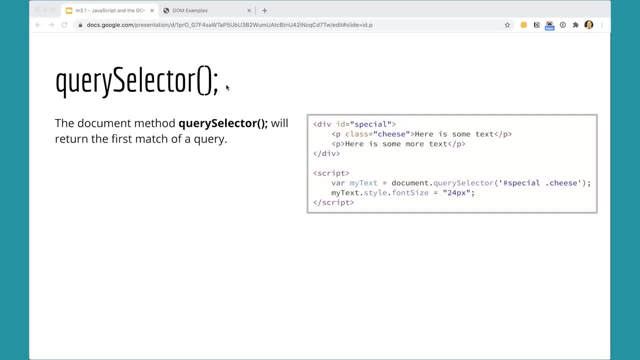 um of a library called jquery. that became extremely popular and it remains very popular to this day- less so now than it was, but it's still a very popular library. that made getting elements in the dom and doing things with them a lot easier, and jquery was very popular for. 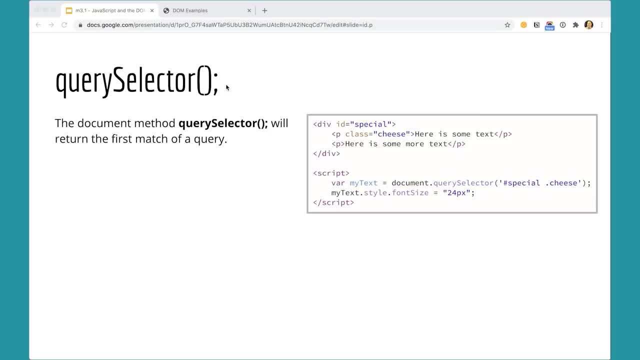 that reason and, um, due to that popularity, uh, javascript had added to it in 2013. so, before es6, an api that allows us to use query selector and query selector- all which we'll also look at- to get elements from the dom, and it's a. 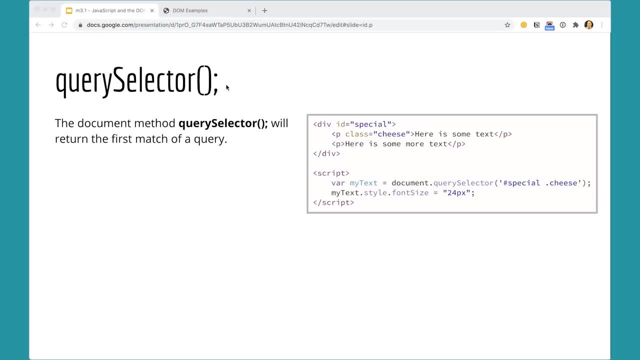 little bit more convenient, but it works a little bit differently than the older get element by id, get element by tag name, get element by class name methods. so these are newer methods and they're very useful, but they work a little bit differently. um, and because of the introduction, 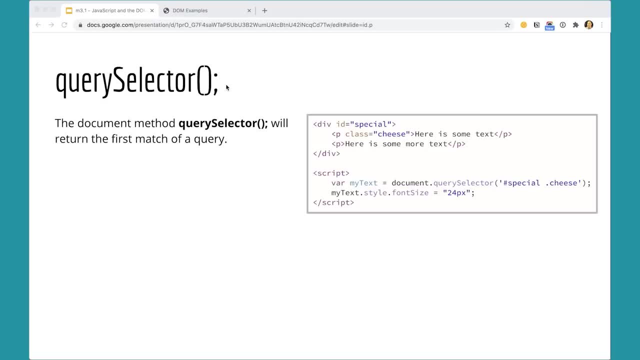 of these methods. jquery is not nearly as necessary as it used to be, and we'll still learn jquery. we'll be learning that in the second course in specialization. but um, now we can actually get elements in our dom a little bit easier than we could just with the older methods. 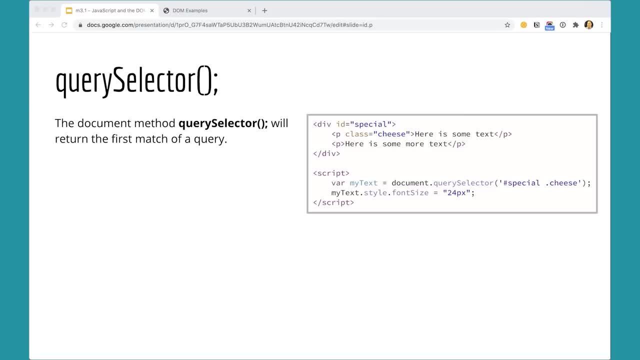 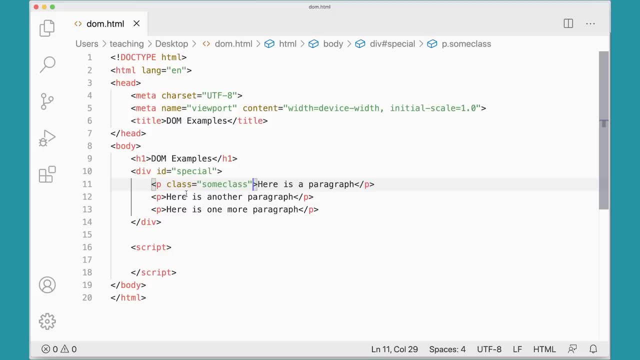 okay, so let's take a look at query selector and the way that works. so over here i have a document and i have a div with an id on it and then inside there i've got a paragraph of the class. well, i could do something like this: um, my var, my text equals document dot. query selector. 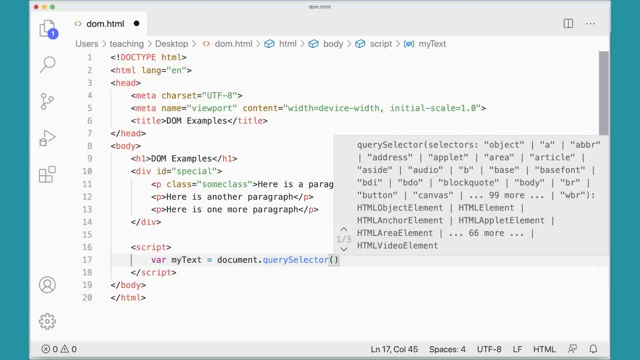 document: dot query selector, and then what i would pass in is actually the instead of just some class. i would put either dot some, i could put dot some class you use the. so what's different here is: before we didn't use the css syntax. now we have to use the css syntax with query selector, or i could even be more specific and i 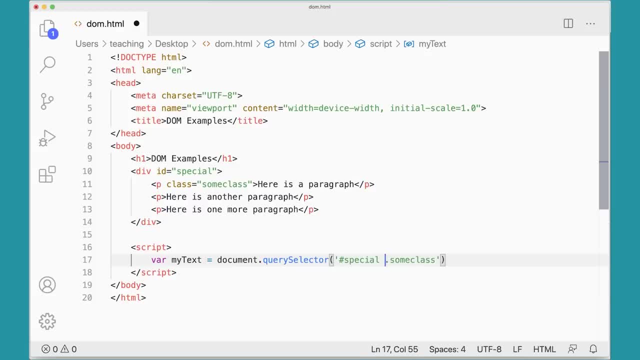 would say: go find pound special, dot some class to get to some class inside the id special. and what's nice about this is that query selector will always return the first element that it finds that matches what you pass in here. so even if i had another paragraph, 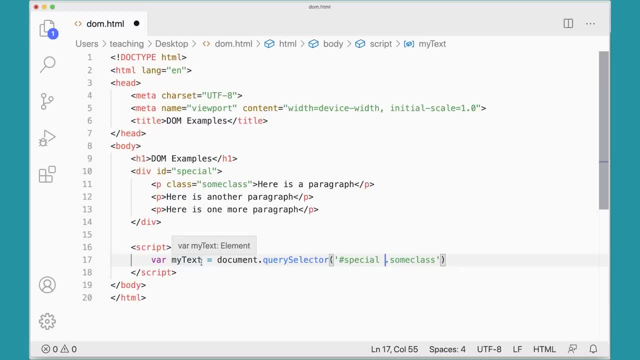 with some class on it. this will always only return one thing to my text. let's put a semicolon there and see if this works. my text dot color of style. dot color equals red and if i go over and test this document again, i recommend that you give this a try yourself. 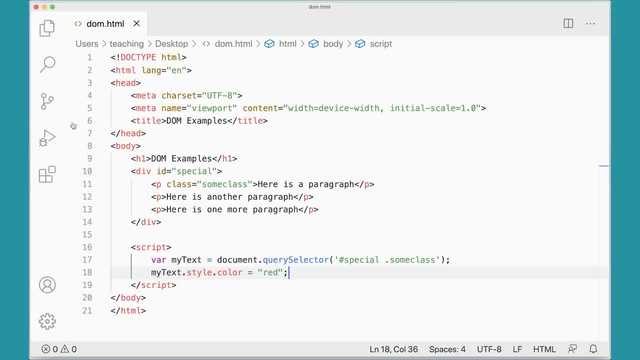 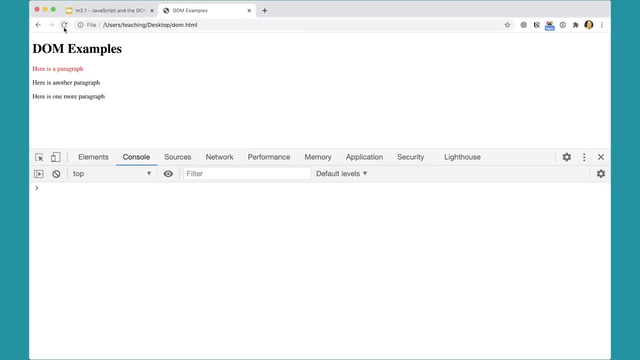 you can see that it's turned that paragraph red. now if i were to go in here and add my class, some class, to another element done on here, like this one here, you'll see it will still only affect the first paragraph if i go back and refresh this, because it only gets the first element. 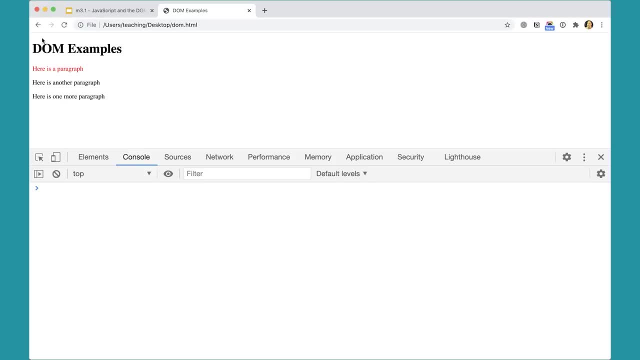 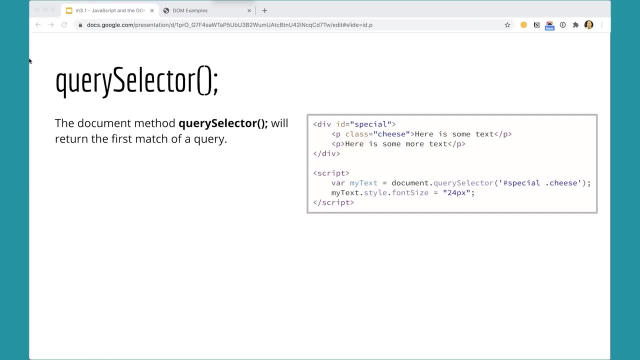 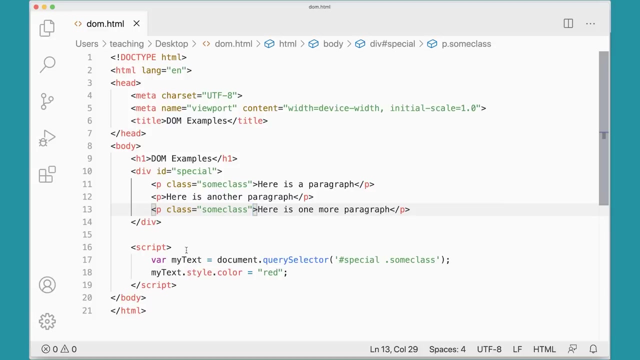 that it matches and that's very useful for when you want to go in and get something like that. and again, remember, with both query selector and query selector, all that you have to pass in. when you pass stuff in, you're passing in the css syntax: pound special instead of just special, or dot some class instead of just some class. that's really. 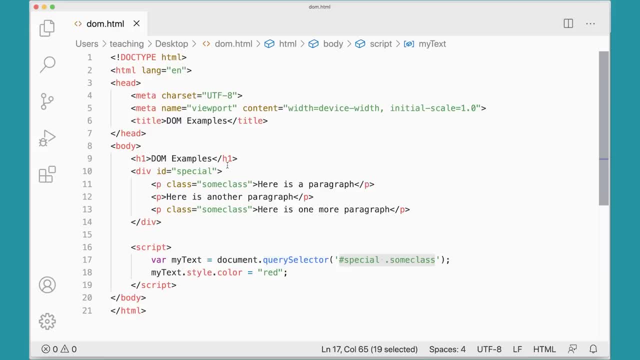 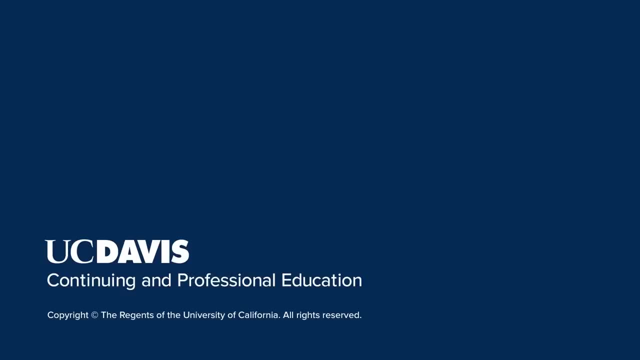 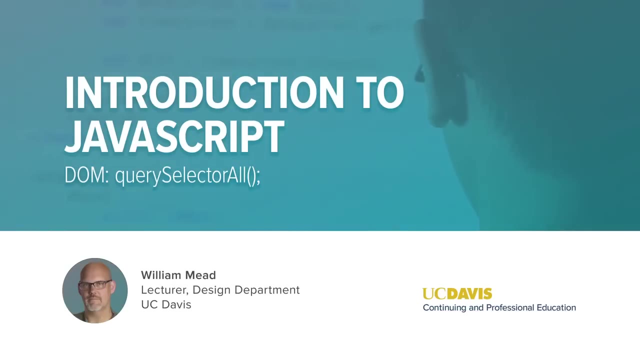 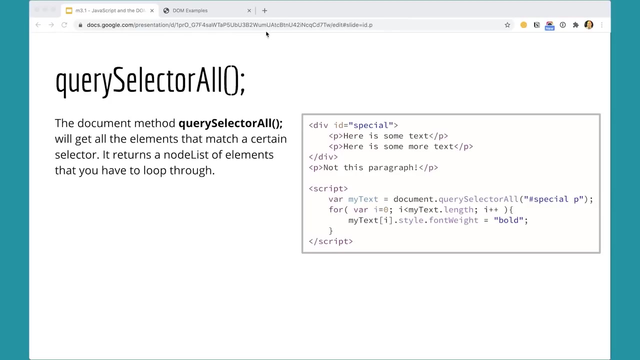 important with query selector. okay, great, let's take a look at the at the query selector all method in the next video. the query selector all method does. what you would think it would do is that it allows you to grab a group of elements again, but this time using the newer, more updated uh dom api. 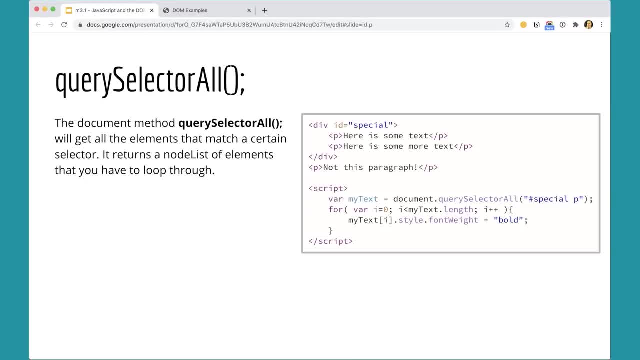 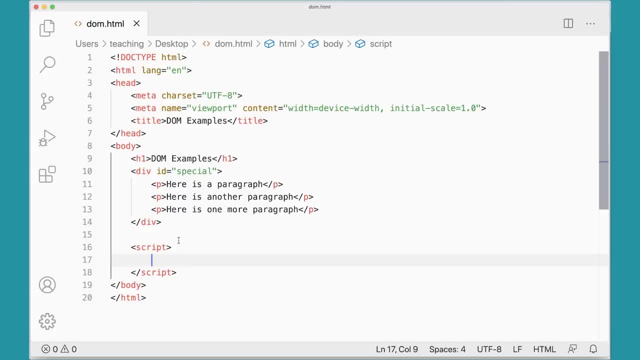 query selector all. so let's go and give that a try really quickly here. so over here i've got my div id special and i've got some paragraphs in here and i can do something like var. my text equals document dot query selector all. i want that one query selector all and i could pass in here in. 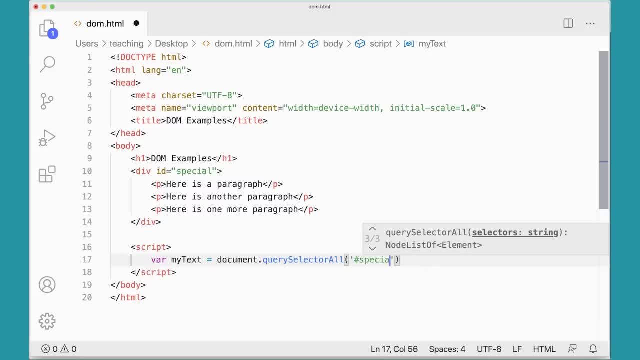 quotes. i could pass in pound special p and that's going to get me all of the paragraphs that are inside this div special so i can go into my document and find a particular group of elements somewhere in my document. but again, with this we're going to need a for loop for var i equals zero. 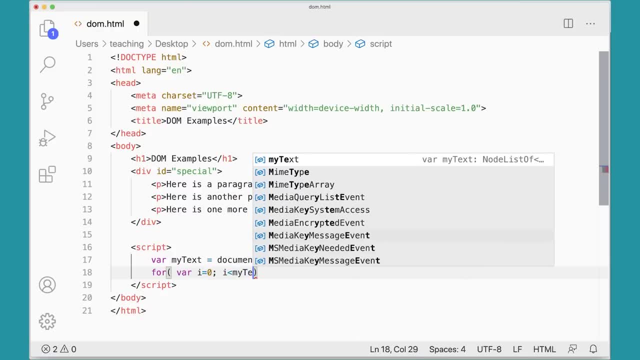 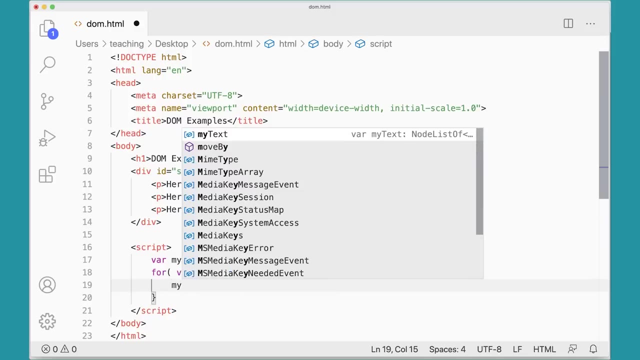 while i is less than my text dot length, i plus plus and then i can do my text square bracket i dot style. dot color equals red. there we go, save that, and then we should be able to test it over here and see when i refresh the page. 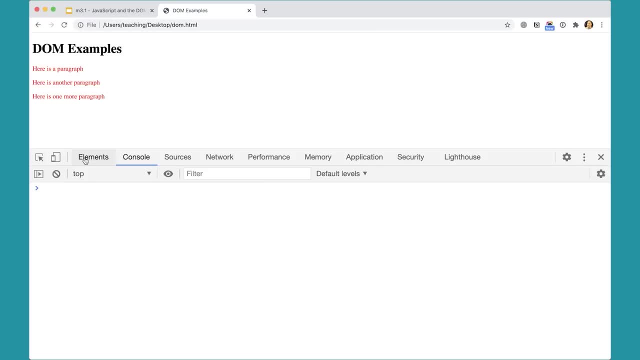 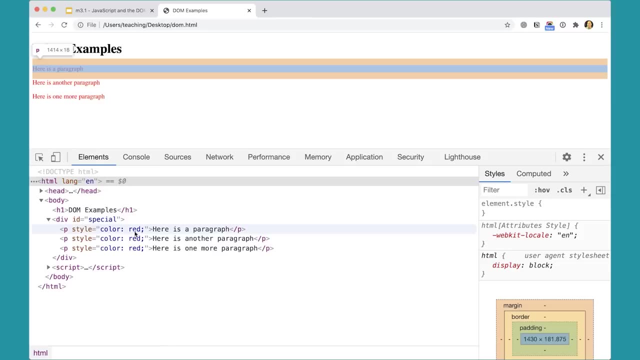 let's. it is turning all those paragraphs red. and just one more time to just drive this home. notice in here: when i go look in that div, it's added style color red to each one of these paragraphs. that's what it's doing. it's going into special and finding the paragraphs and 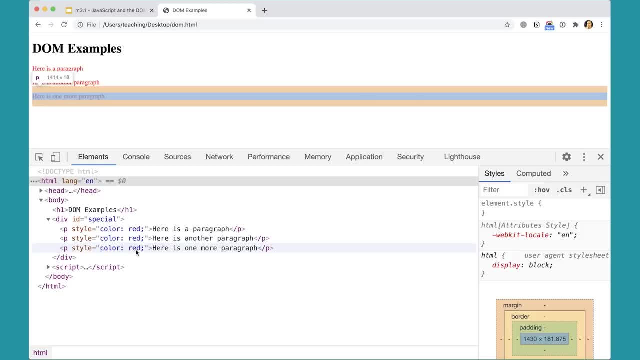 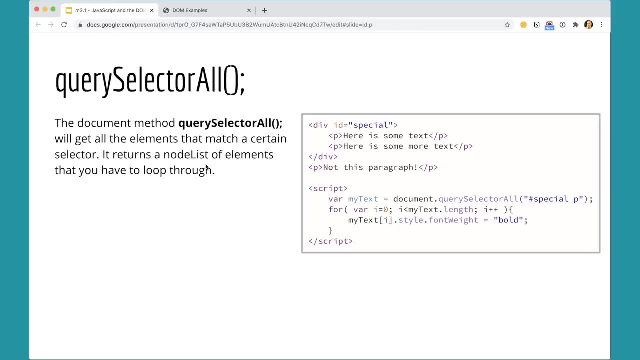 affecting the dom after the page, after the html initially loaded. it's really important to understand that that's the way this works. so query selector all will allow us to get groups of elements and then we would loop through them to affect them one at a time. so far we've talked about five document methods. three of them are older document get. 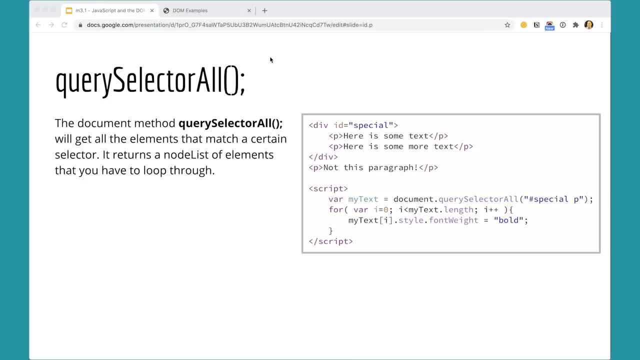 element by id. we'll still use that quite a lot. document get elements by tag name and document get elements by class name. you might use this less often now because now we have the newer methods- query selector, inquiry selector, all. but these are just some of the document elements. 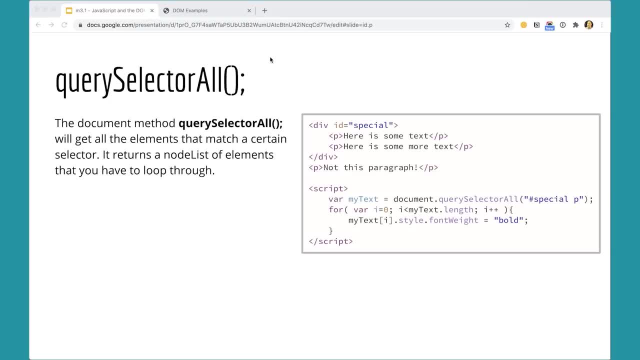 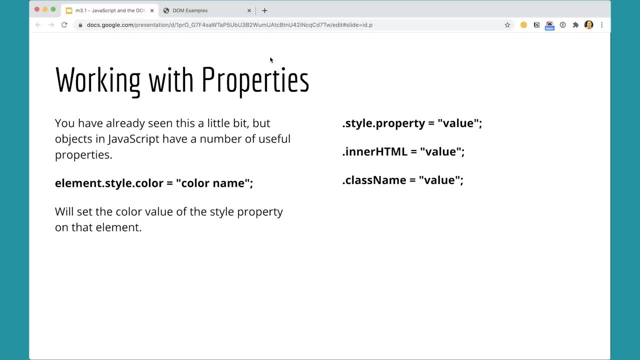 that allow us to add elements to the page. next, i want to talk about working with properties, and we've already seen this a little bit. we've seen elementstylecolor, so we're going in and we're getting that element. whatever the element is, we've got that element, whether it's paragraphs. 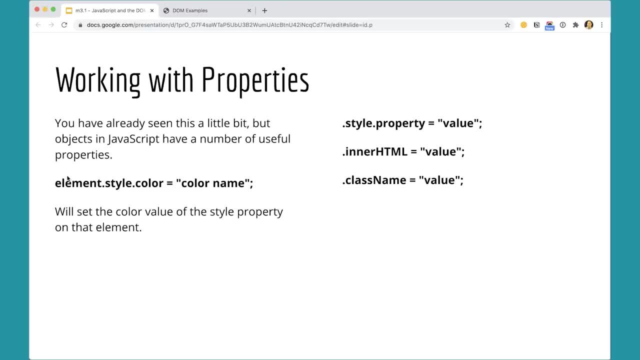 or whether it's a div or whether whatever it is. we're getting that element with our, with our document methods. we're getting those elements And then we can apply the style property. We can get the style property and the color subproperty and set it to whatever color name we want. 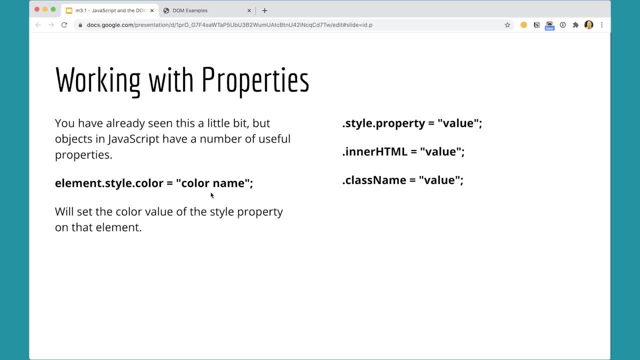 And there are other properties that we can use. There are a number of them. Some of the more popular ones, or ones that we'll use more frequently, are inner HTML- We'll be seeing that one quite a bit, And class name is really useful. 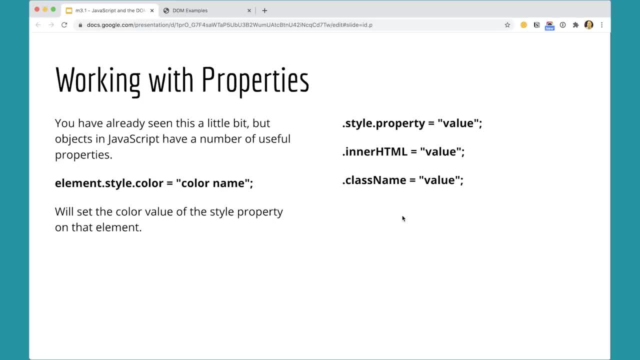 So that you can actually take an element and apply a class to it. This is super useful in modern JavaScript, because CSS has become so powerful. Now we can put animations in CSS and then, when we want to animate something, we can use JavaScript to add that class in CSS. 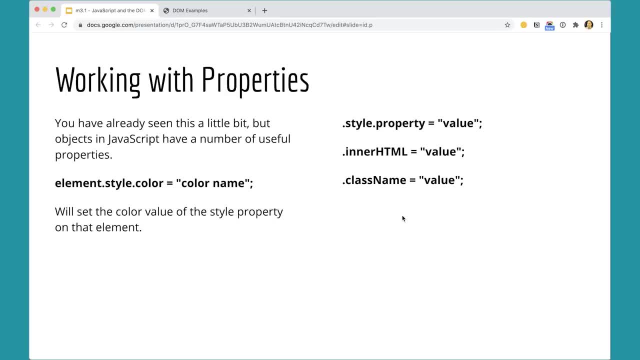 that has the animation, and the animation will take place in the screen, And that's a really, really great way to create interactive or animated elements on a webpage. So we have the document methods and that, and now we have element properties that allow us to work. 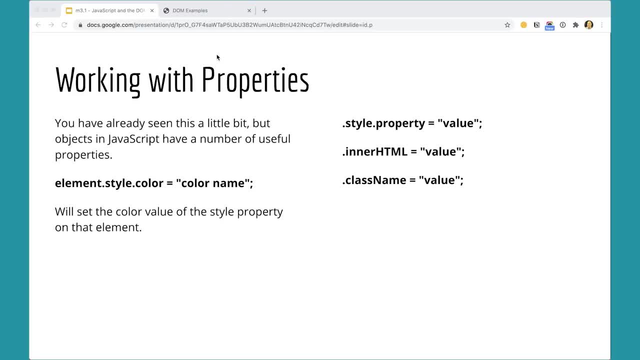 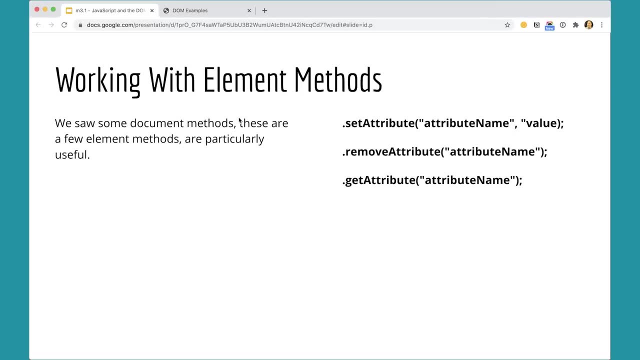 with the properties of certain elements, but there are also element methods or element functions, And those are also really useful. So, for example, set attribute: we can pass in an attribute name and then set its value. So not only can we, you know. 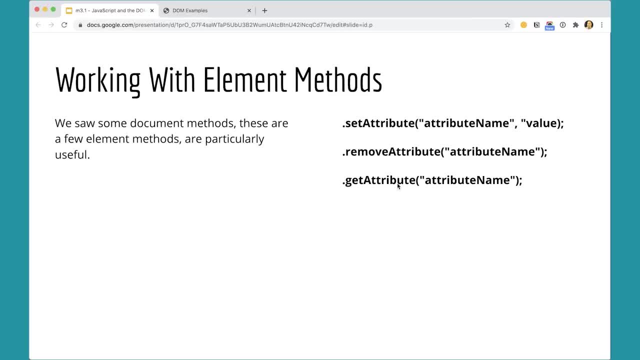 back here we could set the class name by using the class name property. Here we could set the class name by passing in class and then passing in a value. I forgot to quote at the end there, but we could pass in the value there. 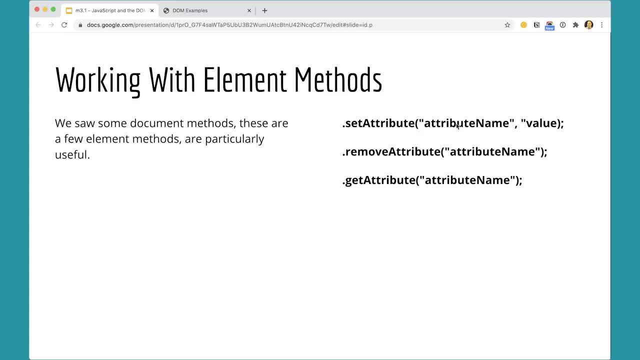 or we could do something else We could use on an anchor tag. we could set the href attribute and set its value, or we could remove an attribute, or we could get an attribute and do things with it. Notice that methods are distinguished by the fact. 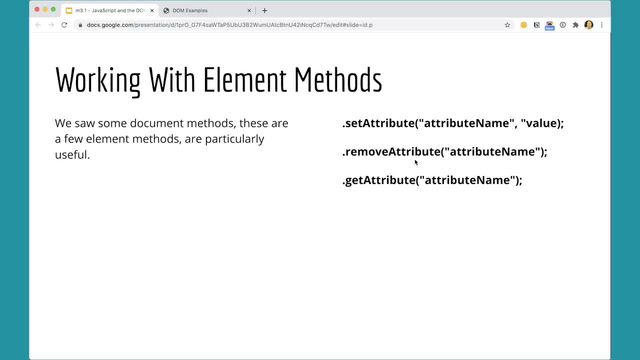 that they have parentheses. So when you're using a method or a function, it has parentheses, whereas the properties don't have parentheses. They have an equal sign and then the value. So that's how you can tell the difference between a property and a method. 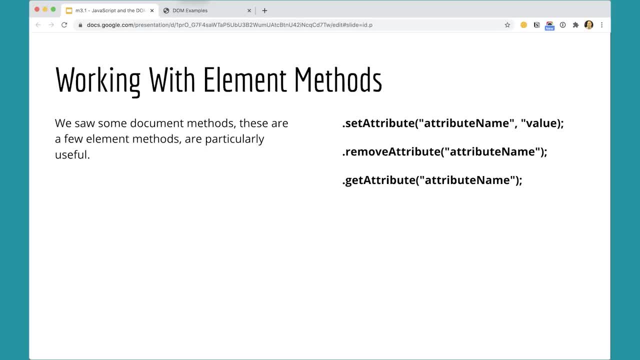 Okay, great, Let's see what else we can do with this. This may be a little bit confusing at the moment, but I promise- so that you'll be able to see this- that as we practice this stuff it'll start to make more sense, but it does. 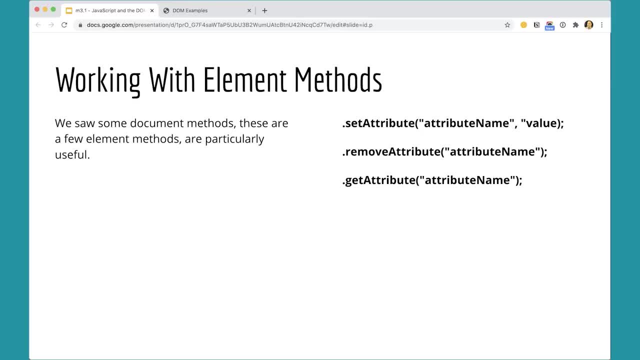 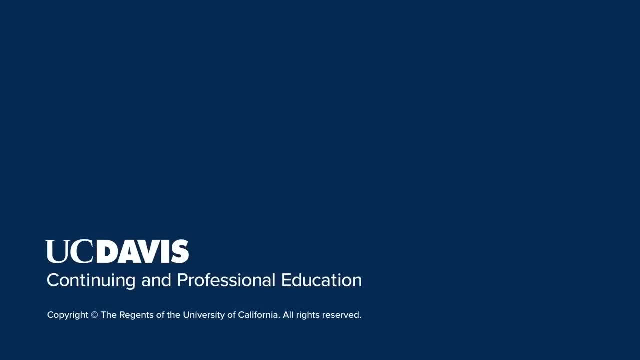 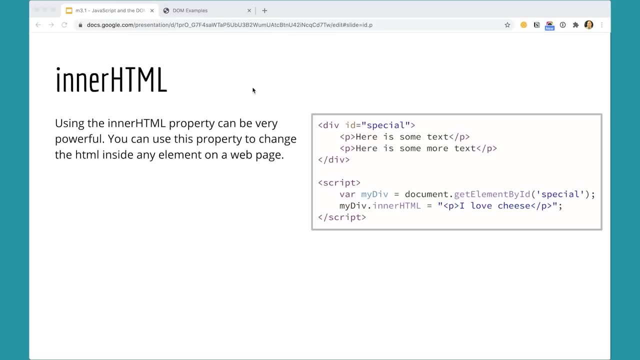 take a little bit of getting used to all these methods and properties for working with our document to to affect your web pages. next, we'll take a look at one of the element properties that we just talked about in the previous video and see how powerful it is, and that's inner HTML, and. 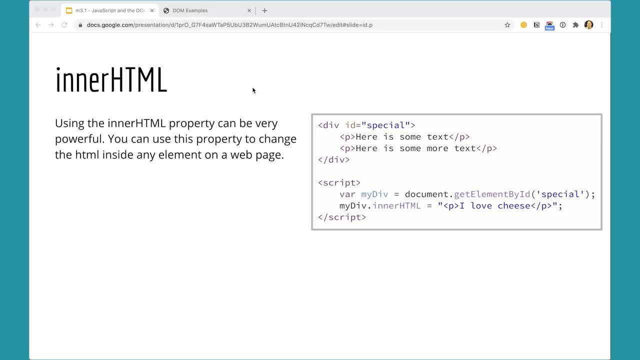 if you look at this image here, you can see I have a div with an ID special and I can use any of my document methods to go in and get that div and then I could use inner HTML to actually change the contents in that div. I can replace these: 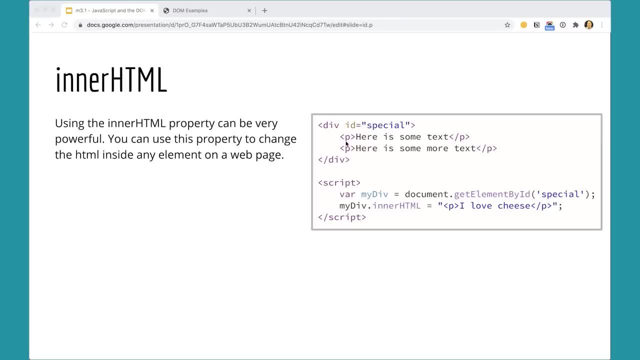 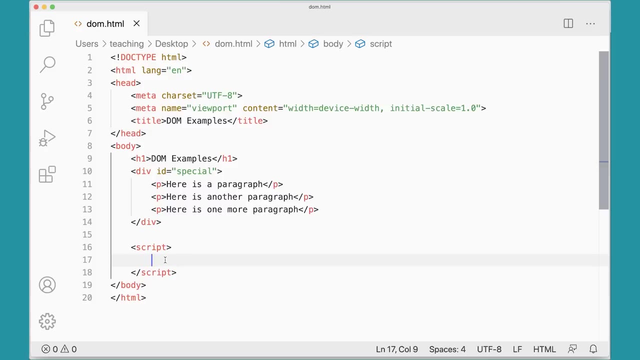 contents with something else, entirely, completely new, completely different, and that something else could have HTML in it. so let's see what that looks like. so over here I have my div ID special. I have these three paragraphs in here, but down here I could say: bar, my div equals. 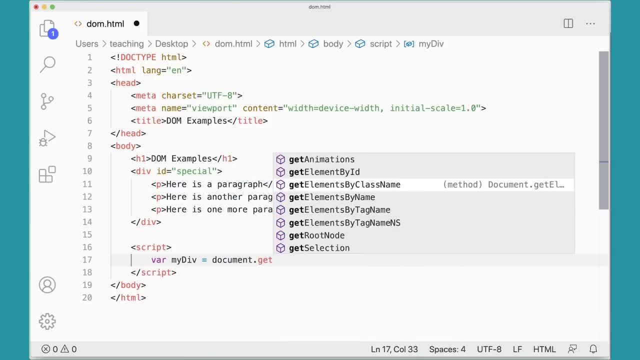 document dot: get element by ID. pick it from the list so you don't spell it wrong. special with this version: we're not using the pound here. we're using the older get element by ID. we can switch that in a minute, just to see what that looks like. 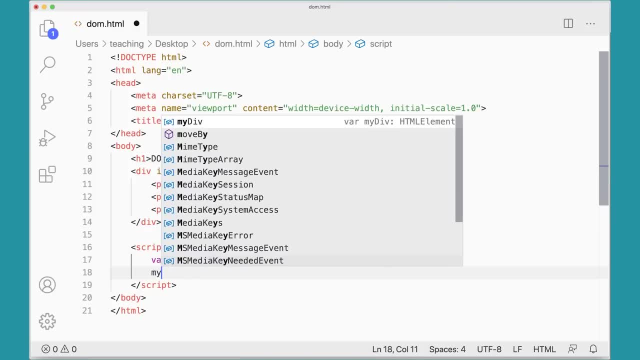 but then I can say, okay, I've got that element. my div dot inner HTML equals: this is an element property, so we use the equals sign and then inside quotes I can create a completely new piece of content to stick in there. okay, great. so now when I run this you'll see over here it's still bread from. 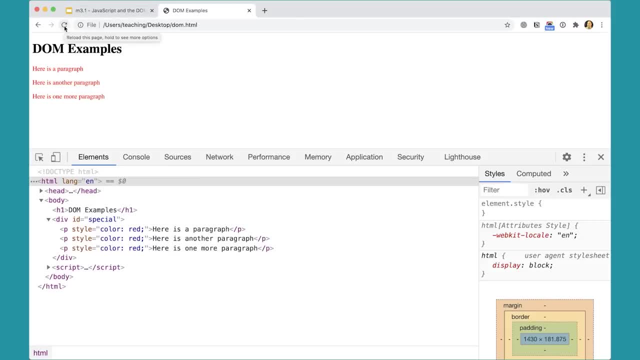 before. but that's okay, those paragraphs are going to get removed and replaced with the new paragraph. look at that. and And if I come down here and look and inspect in my body and look at div ID special, there's only one paragraph in here in my inspector, Whereas if I were to do view page source, you'd see three. 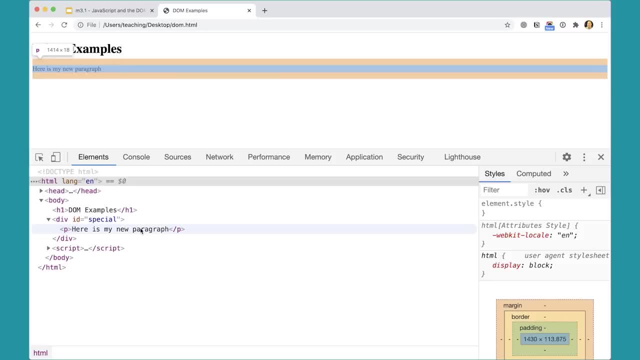 paragraphs in there, Because when the page loaded it had three paragraphs And then the script ran and it removed those three paragraphs and put this one in instead. And that's what JavaScript is doing. And I can't express how powerful this is, Because frequently what we need to do on our 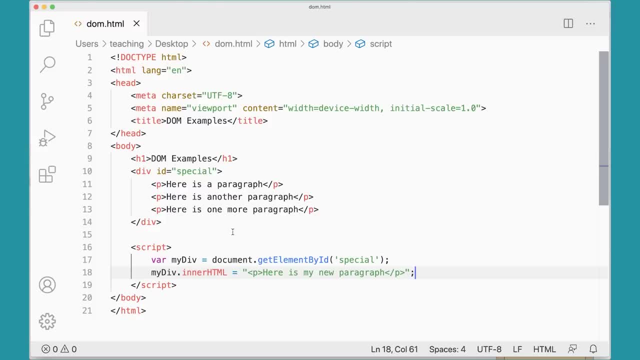 web pages is: take a bunch of content and replace it with some other content. Now here I'm using get element by ID special. I could also do query selector, But if I use this one then I would pass in pound special. You see the difference there. 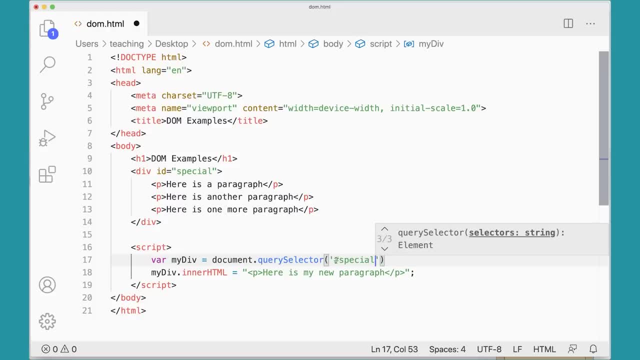 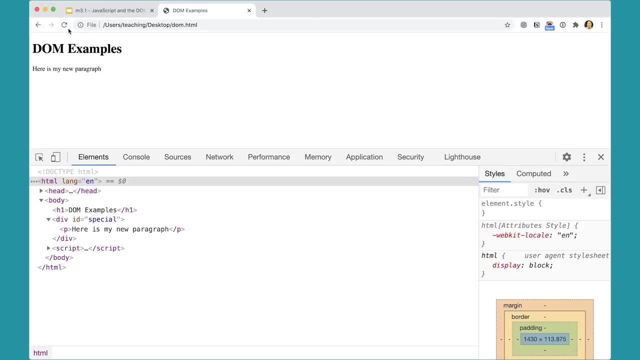 This is the newer method and it uses the CSS syntax to get to that element, But this will work just the same. I go back and refresh this page. you'll see. it'll do exactly the same thing. It'll get my new paragraph and put it in there, So you could use whichever document method you want Once. 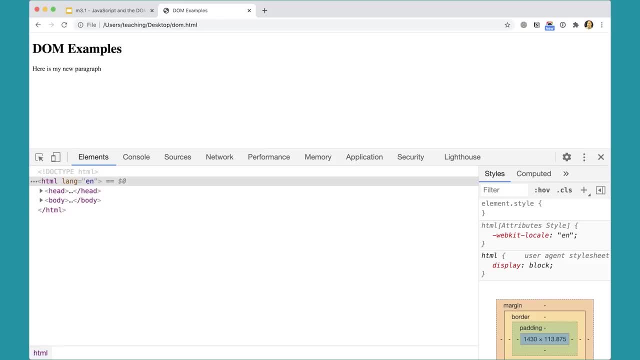 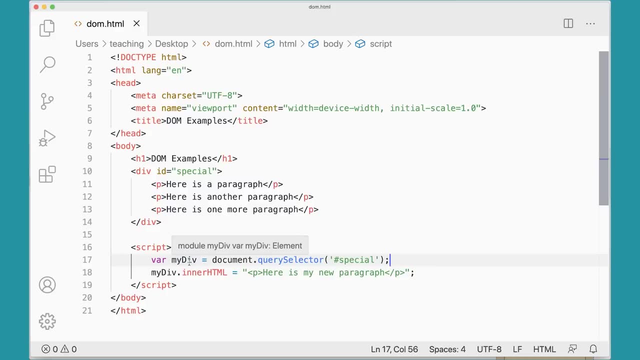 you get that element, then you can use your element properties to affect the element here. Now I'm putting this all inside of a inside of this div here, But you know I don't need to use the variable, I could just do document. 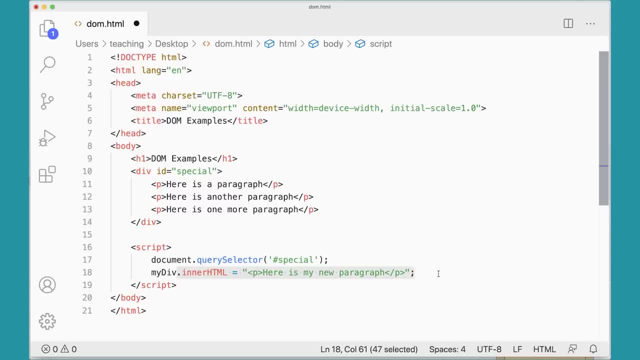 get element by ID special and then put this here. it just makes for a very long line. So it's it's kind of helpful That'll work. It's kind of helpful to have the variable, but you don't have to have. 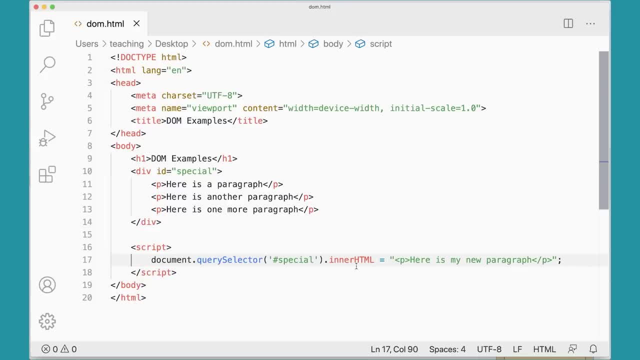 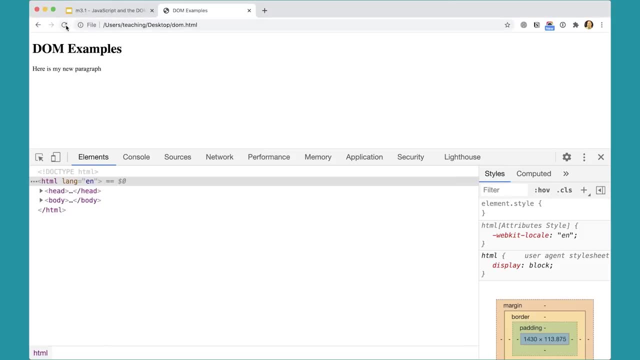 it. I can just go document, I can just go to my next topic here. go to the next is my next item here And I'm going to put that query selector special dot inner HTML And then set my property right there. 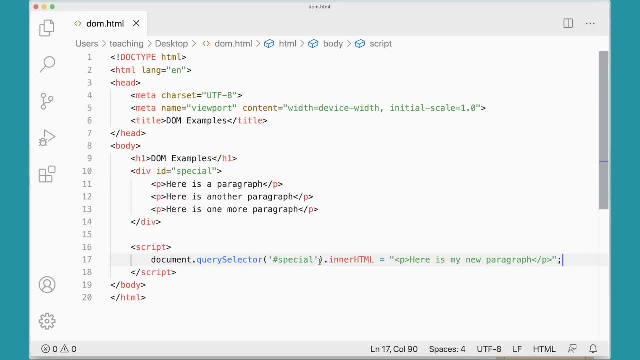 And that'll work just as well. So that's using the inner HTML, And again, I just cannot over emphasize how powerful inner HTML is. we could use this in lots and lots of places to get elements on our page and then replace it. and then replace it with the new main posit het v1 html. whew, whew, whew, whew, whew, whew. a lot of work over here, But anyway, I guess that's the end of the review And hopefully this was helpful. Please give us a thumbs up if you enjoyed it. Thank you for watching. Take care of yourselves and we'll see you in the next video. Thank you for watching. Bye, Bye-bye. 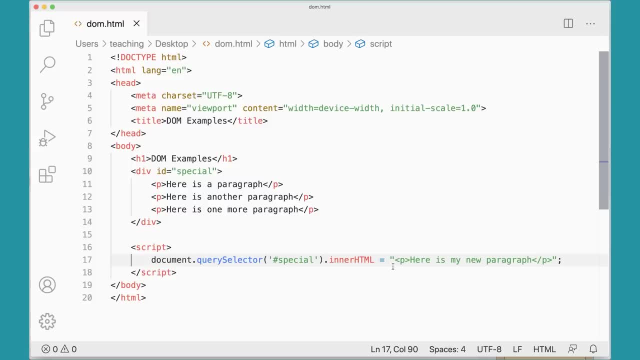 those elements with completely new elements and you can put more html in there. we could put an entire document of html inside this div, not just one paragraph, but you could put articles. you could put all kinds of stuff, images, all kinds of things could go in there using inner html. 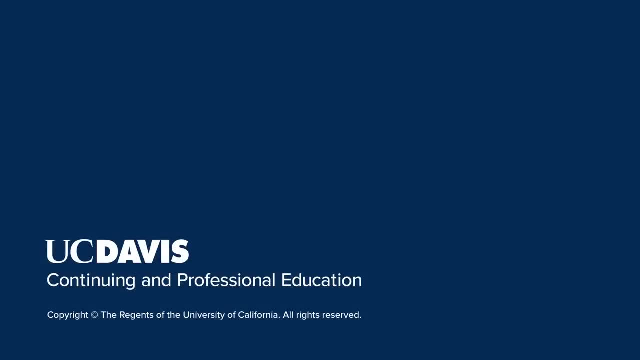 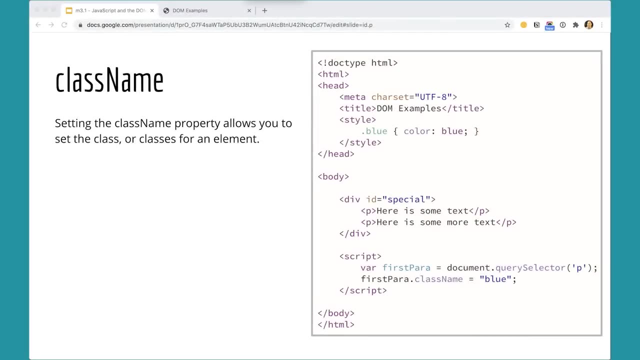 the next element property that i want to show you, which is extremely useful, is the class name element property, so let's take a look at how this one works here. i have a div with some paragraphs in here and i'm using my query selector to get the first paragraph because, remember, instead of 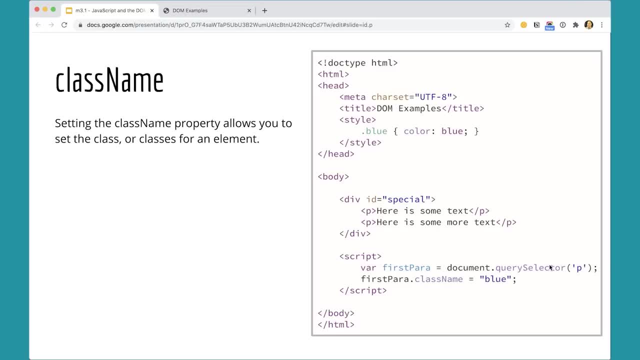 returning a class name. i'm going to return a class name and i'm going to return a class name. collection query selector returns the first one that i find, so it's going to go in here and look for the first paragraph and then i'm going to take that first paragraph and i'm going to use the. 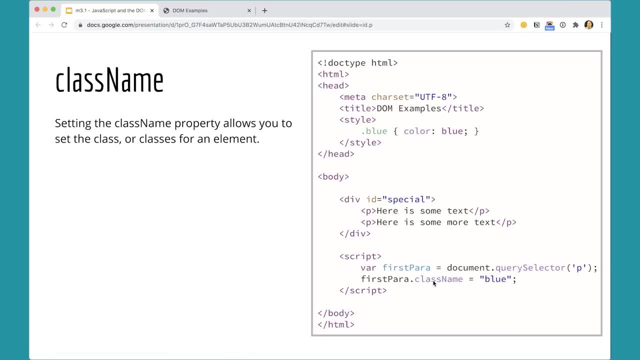 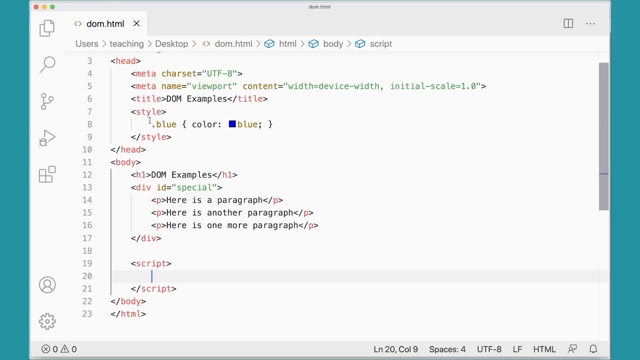 class: name property, element property- to set the class to blue, and up here i've added style and i've added a class blue here to my document. so let's see how this works. i'm going to go over to my page over here and you can see i've added up here a rule here to set. 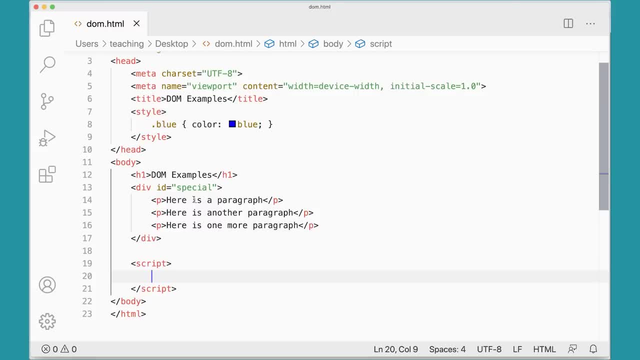 for anything that has the class blue here. so let's come down here. i'm going to call this var first. para equals document dot query selector. and remember we have to use the css syntax. in this case it's just a p because it's just a tag selector. 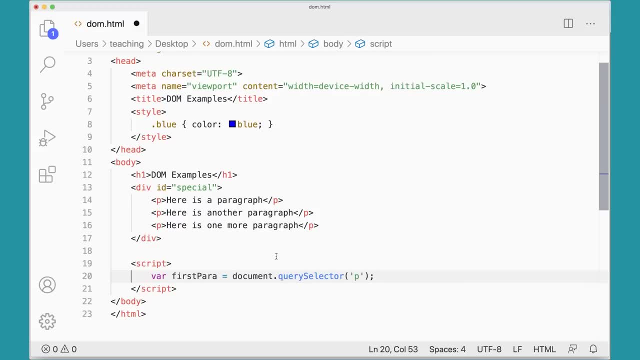 but i'm going to go get that first paragraph. now i've got three paragraphs, but remember i selector just returns the first one and then i'm going to say, okay, first era, set the class name. and you can see here there's one called class list. i'm just showing you a few of the uh, the document. 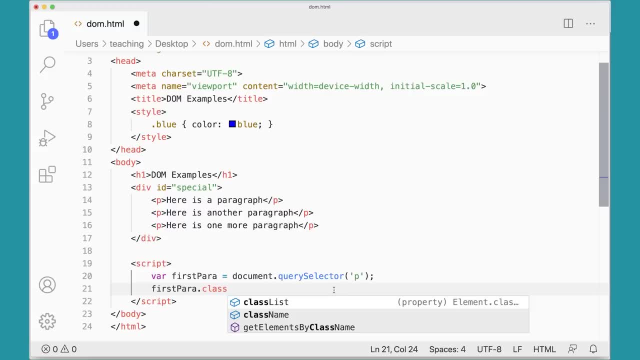 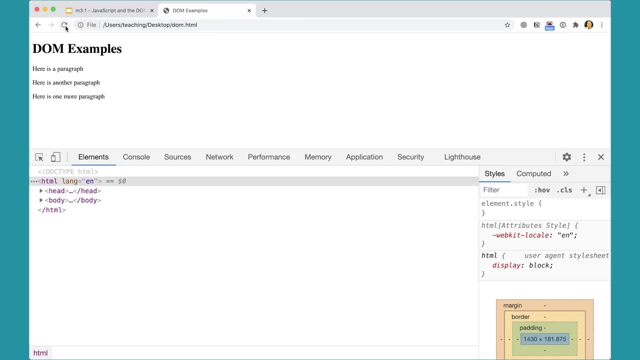 select the the document properties that are super useful, but there are plenty of other ones that you can look up and work with as well. class name equals blue. so now, when i run this, come back here, click on my document. here i've got my three paragraphs, but when i refresh the page it turns the first paragraph blue. and if i come down here and look, 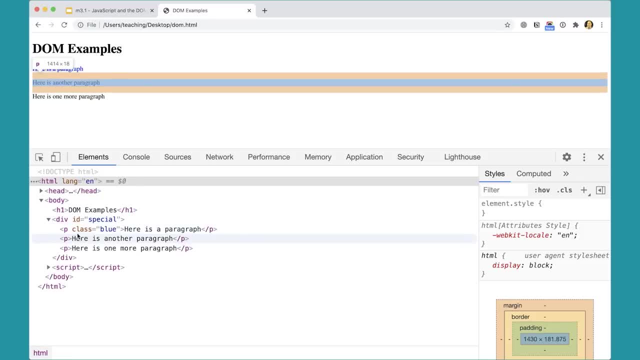 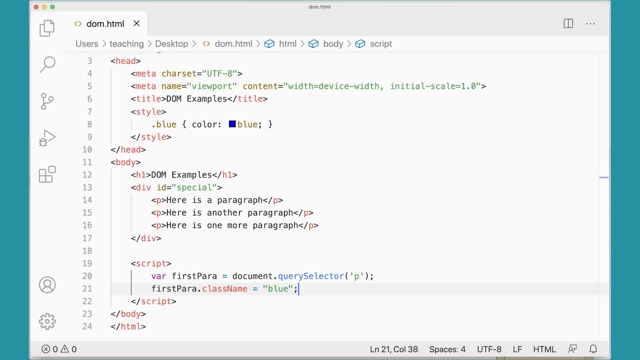 at this. what is it actually done there? but it's added class equals blue onto that paragraph. sure, i could have set the style color property to blue, but adding the class blue is even more powerful because even though in both cases i'm just setting the color, i could have a lot more declarations. 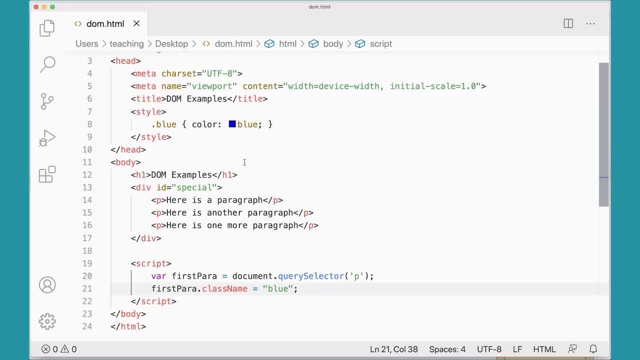 in this class up here. that would do all kinds of things that i could be adding in animation. i could be doing all kinds of really cool stuff, and we'll get to do some of those things in this course. so so hold on to your hat, because it's coming um. 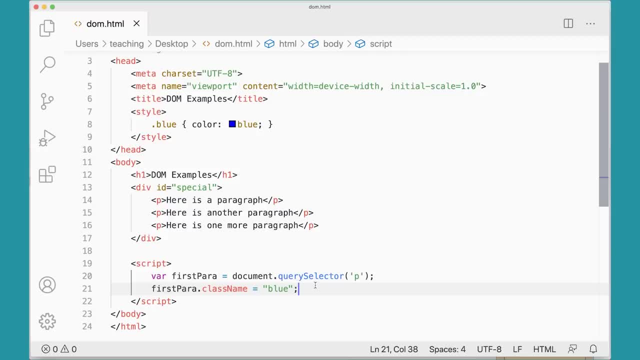 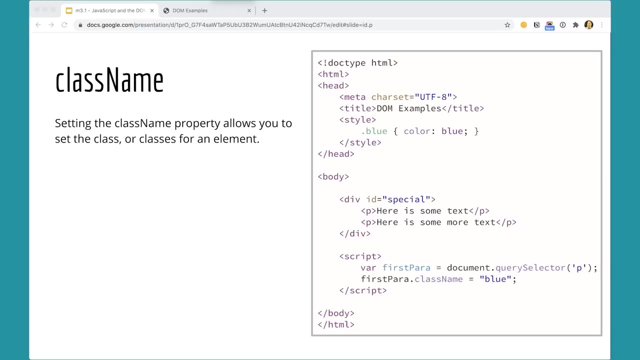 but first I just want to introduce the basic concepts. to begin with- and this is a super useful one- using the class name property to set a class that already exists on the page. it's just really, really powerful. back to our slides. here we've looked at a few of the element properties that we can set: the style. 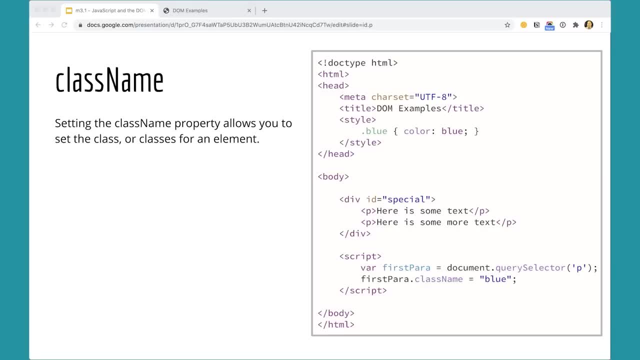 property with the sub properties for our different CSS features. we can use that one. we can use the inner HTML property. that's extremely powerful for replacing HTML inside of any element. and then there is the class name property. that allows us to put a class name on things. the next thing I want to look at: 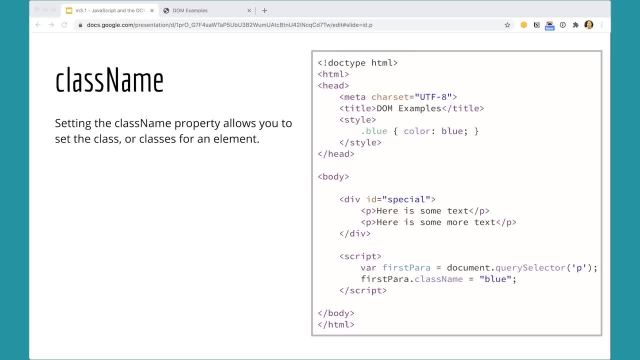 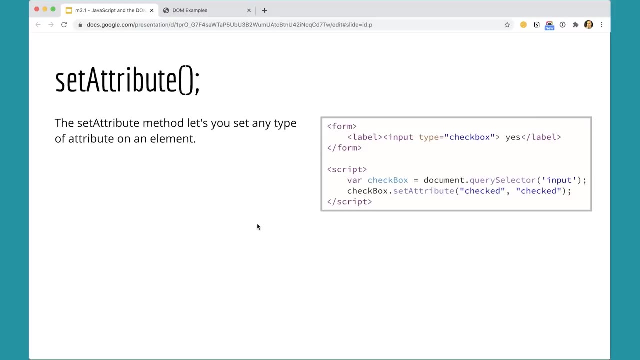 really quickly is some of the element methods. remember, these are properties, because they've got the equal sign and then a value. but we also have element methods, and the first one we'll look at is set attribute. so here I have a form and let's just do this one really. 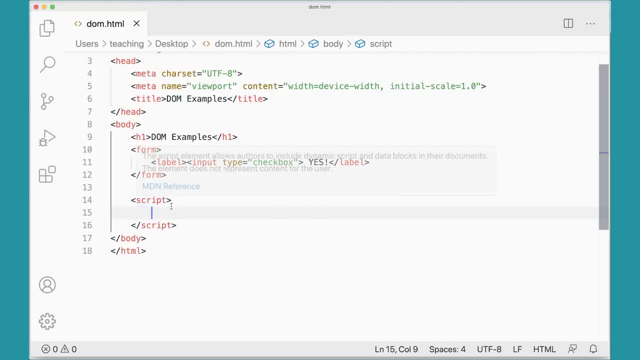 quickly here I have a form and I'm going to say: bar, my checkbox equals document: dot get elements. I can do query selector, query selector input, and then I'll get my first input field here and then I could do: okay, my check box dot set attribute and set. 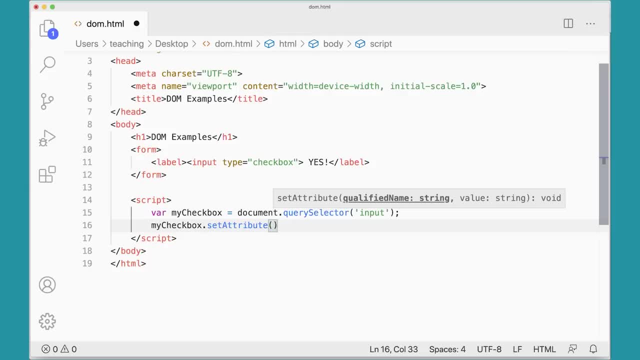 attribute takes two parameters. I'm going to say what is the attribute that I want to set and where do I want to set it, minus two, except for one I can even use. In this case, it's checked and I'm going to set the value, which is also checked. 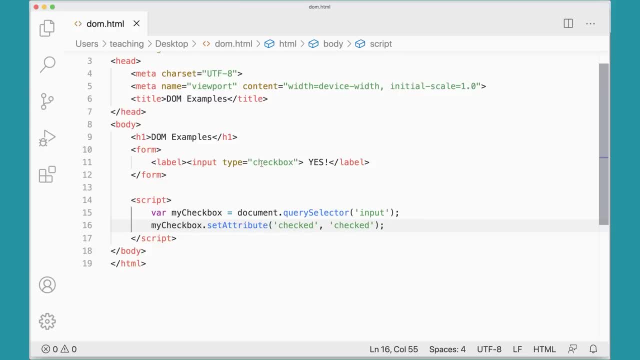 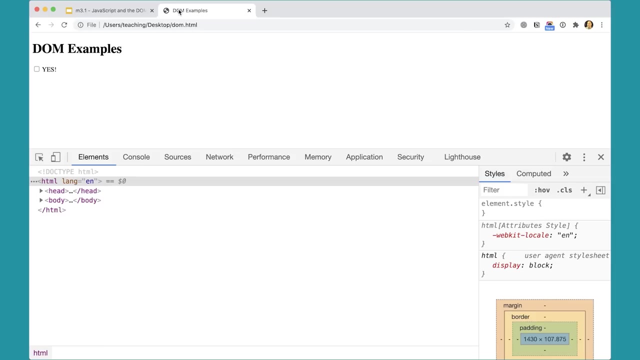 Checked, checked, and that's the way. What that will do is it'll come in here and it's going to set a checked attribute and set it to checked, which will make the checkbox checked by default If we go over and view the page currently without having set that checkbox. 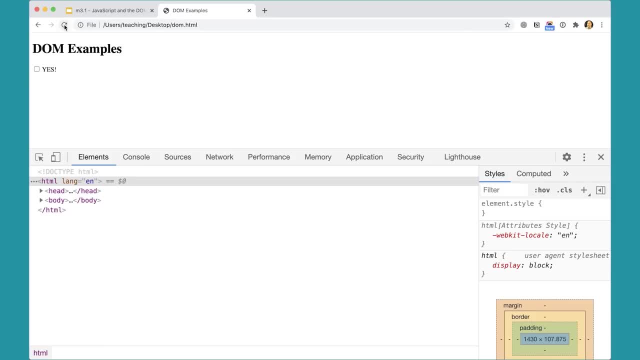 you can see. I've got a checkbox here, but it's not checked. When I refresh the page it comes up as checked by default. If I come down here and look at this, you can see checked equals checked. It's added that attribute into my HTML here. 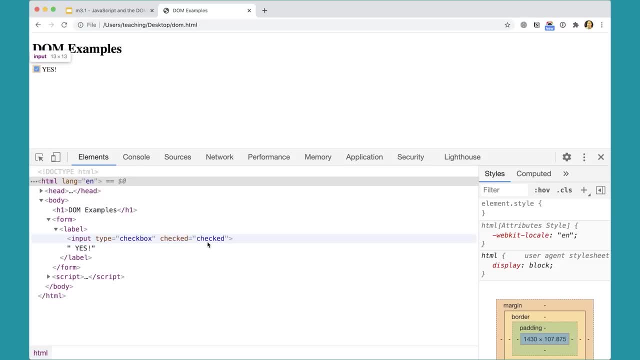 Set attribute can be used for any number of attributes. You want to set an image source on an element? you could use this. You want to change the href on a link? you could use this. Any attribute could be accessed with set attribute. 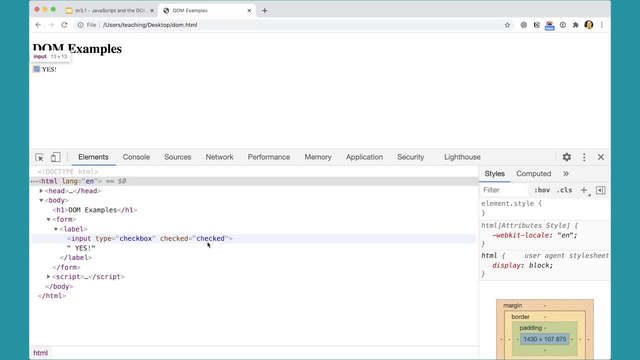 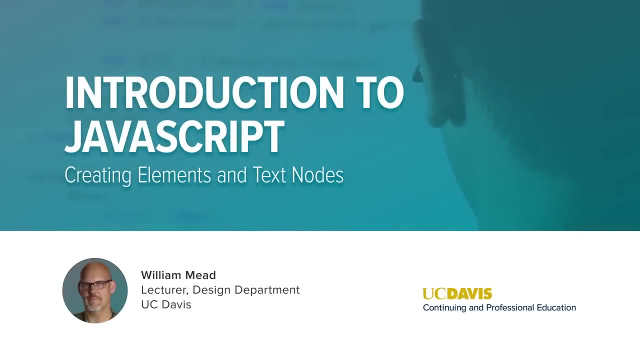 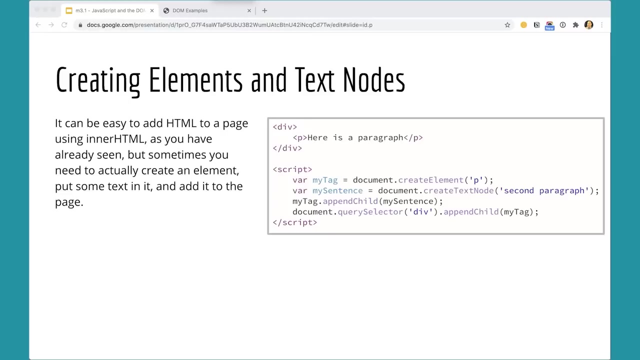 and you could set it to whatever value you want to set it to. That is another very powerful tool that allows us to change content on our webpages. I have shown you a few of the document methods, the element methods and the element properties in this lesson. 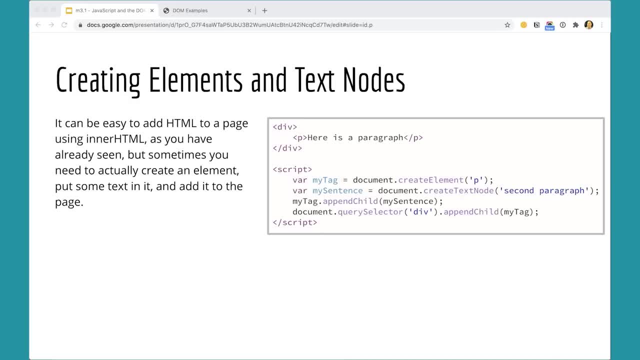 There are lots more. There are many, many more that you can use to do all kinds of interesting things to your pages. I think it's helpful to see just a few to begin with, to see how those work and to experiment with those in a limited way. 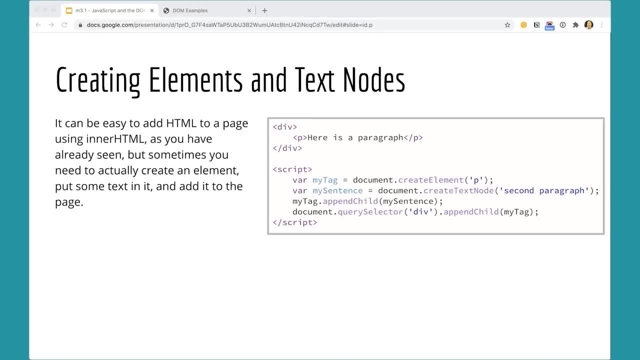 Then add more, Add more features and methods and all of that stuff as you go along. I do want to show you just a few more in this lesson, just because I think it's helpful to just see that there are different ways of doing things in JavaScript. 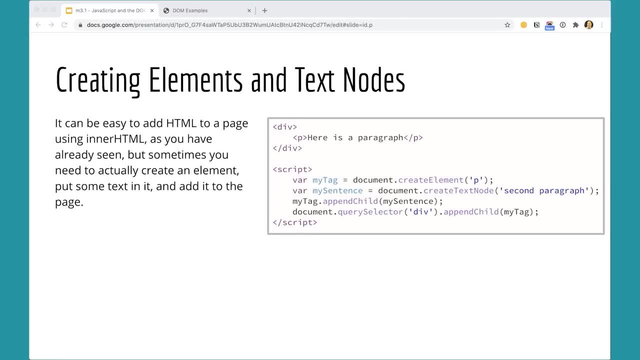 And this one I want to show you is a way of creating elements and text nodes in JavaScript and then adding them to the page. It's kind of an interesting process And again, we've used inner HTML and we can use that to also change content on the page. 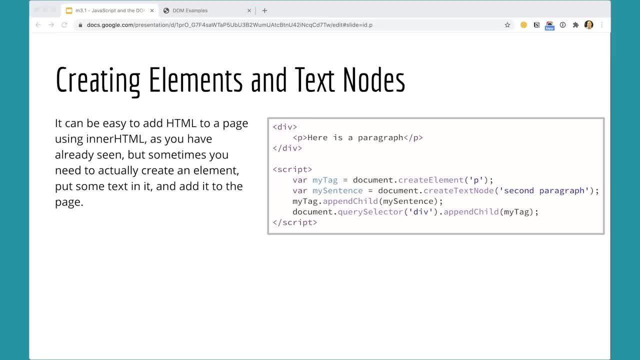 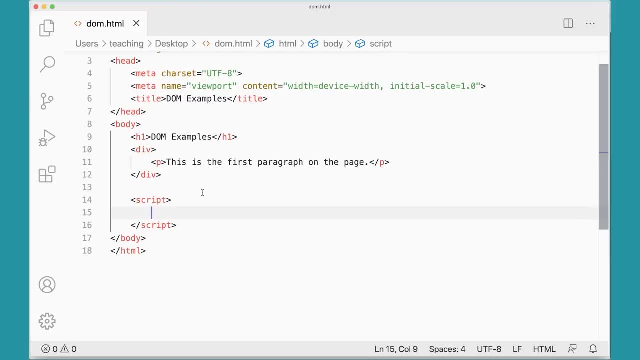 But this is just a different way of doing it. So here let's actually switch over to the code editor so we can actually do this. Here I'm going to make a variable, var myTag, and I'm going to say documentcreateElement. 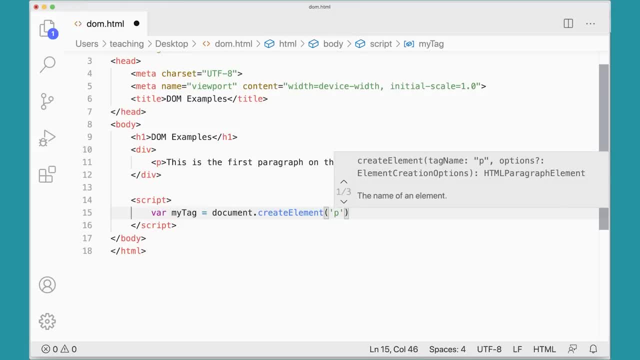 Create an element. And what am I going to create? I'm going to create a paragraph, So this makes a new paragraph And puts it into myTag. createElement is a document property that makes a new element. And then I'm going to make a new text node. 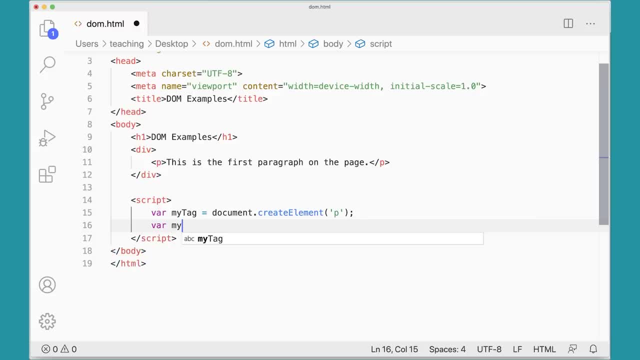 var myText equals documentcreateTextNode. Here's a new paragraph, So I'm going to make the text node. So JavaScript creates a text node. We create the paragraph, We create the text node, And then we're going to say myTagappend child myText. 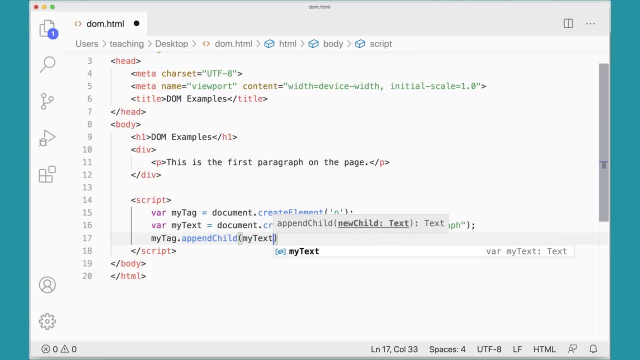 So that takes the paragraph that we just created- the text node this text- and sticks it into the paragraph tag that we've created. So all of this is just happening in memory in JavaScript, And then we have to actually put it on the page. 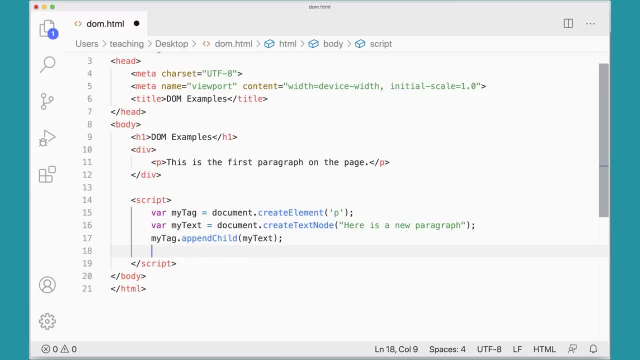 So I'm going to get my div here: var- myDiv, var. myDiv. var. myDiv equals documentquerySelector div. That's going to go find the first div on the page And then I can say myDivappend var- myDivappendchild- myTag. 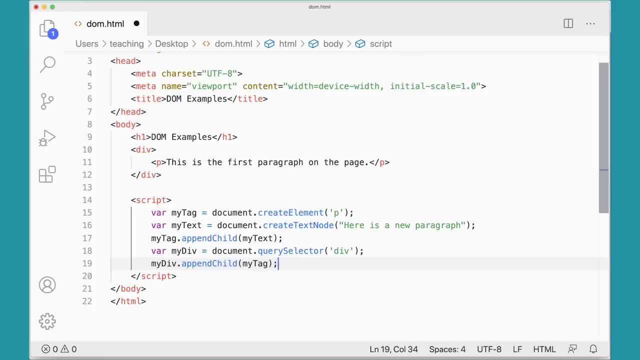 So we're doing a multi-step process here, where we're taking the paragraph, we're creating a paragraph, we're creating some text, putting the text in the paragraph and then going and getting our div and putting the paragraph, appending it to the paragraph. 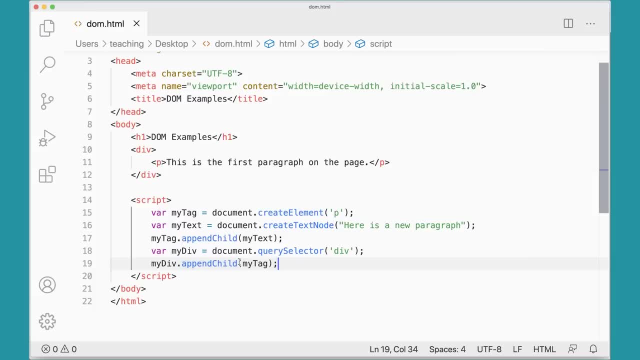 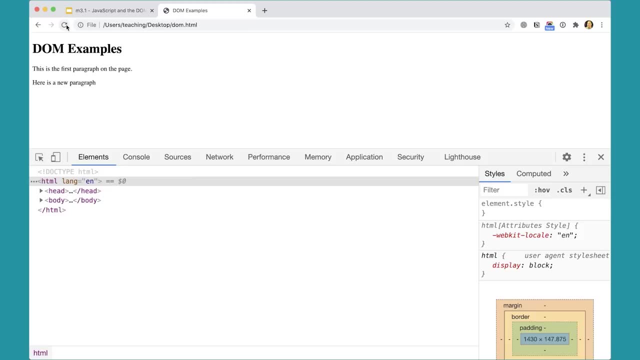 And then appending it to the end of the paragraph there. Let's see if I did this right. If I come back and do this over here and refresh, you can see that my first paragraph is here and a new paragraph has been appended inside the div. 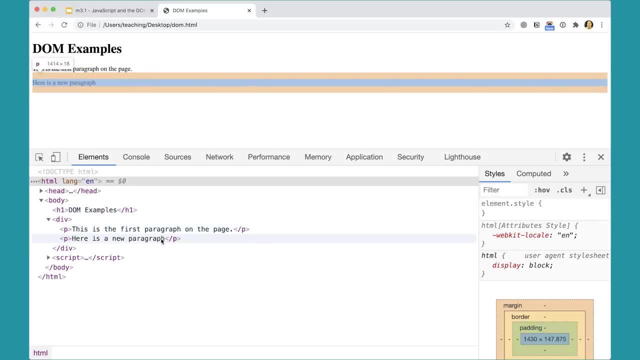 It's been added to the div here And JavaScript is doing that through this process. Could I have just used interface? Could I have just used inner HTML and added and changed the contents of this div so that it had these two paragraphs? Sure, I could have done it that way. 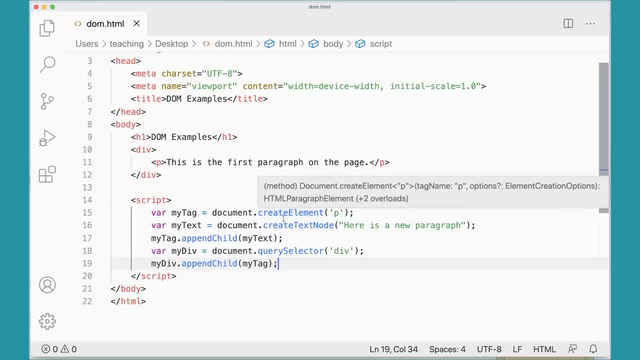 But sometimes it's useful. This seems like a kind of convoluted, complicated way, but sometimes it's useful to actually create the elements using the document method, createElement, to create content, to stick in those elements and then to append them to the page in particular places. 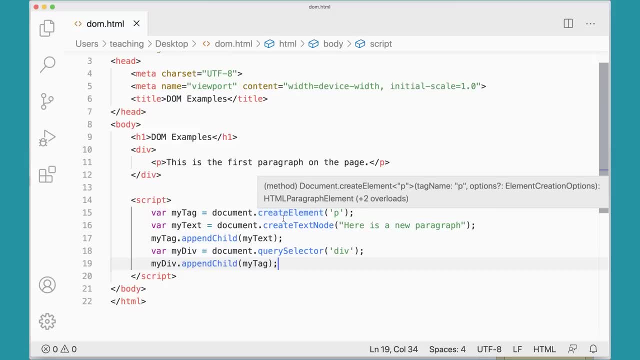 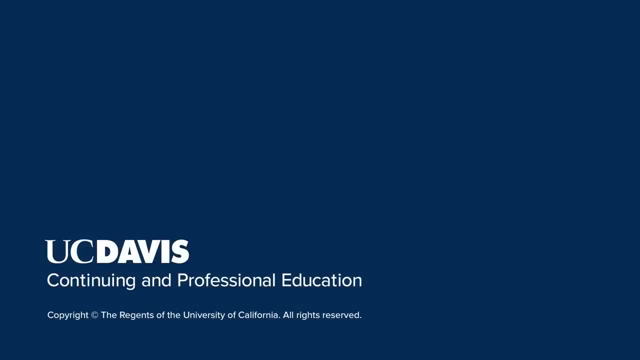 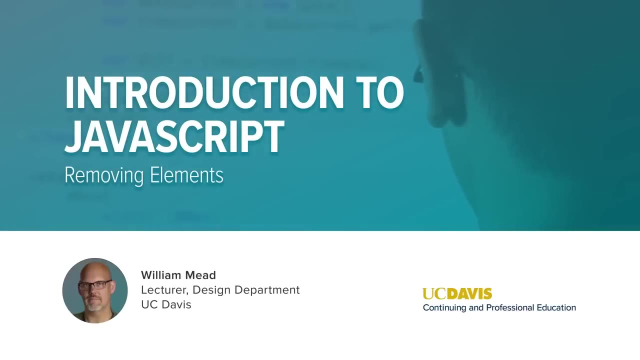 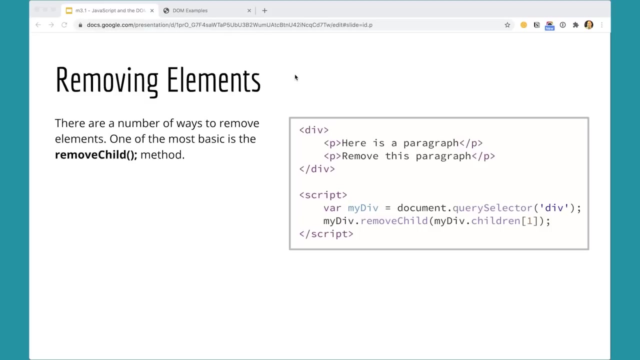 Sometimes it's useful and sometimes a better way to go than using inner HTML in certain circumstances. One last method that I want to show you in this lesson is how to remove an element from another element, And again we could use inner HTML and just replace all the contents. 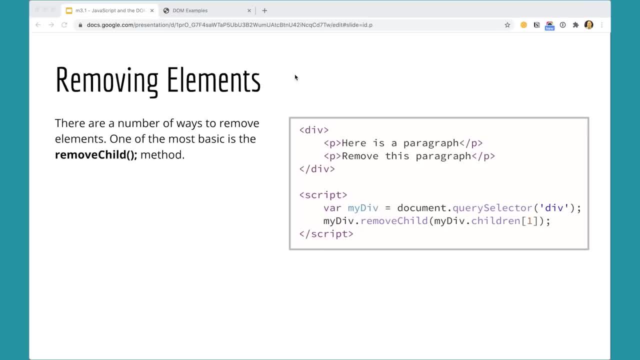 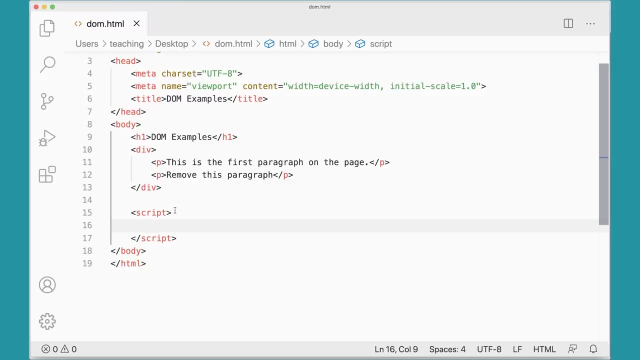 all of one element, But sometimes removing elements is useful. So let's take a look at this example really quickly. Here I have a div with two paragraphs in it And I'm going to go ahead and get that div and put it into a variable: var myDiv. 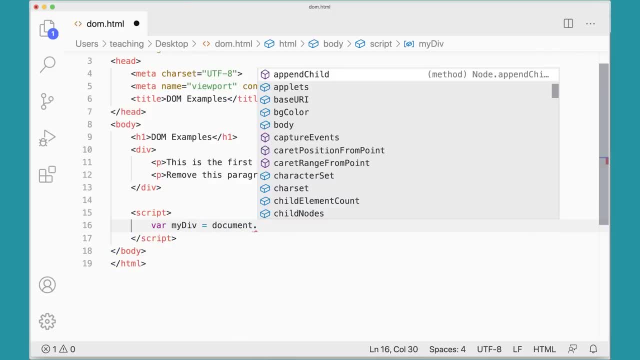 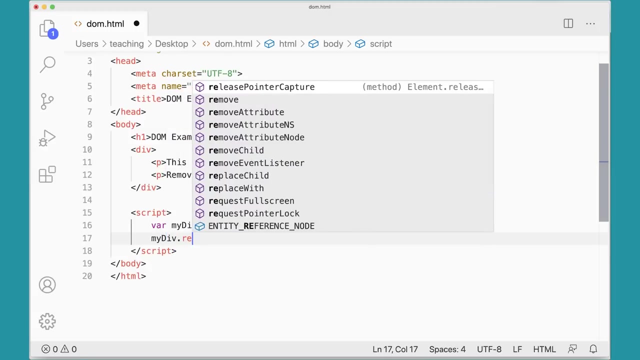 and assign it documentquerySelector div. That'll go get the first div on the page, which there's only one, so that's nice and easy. And then I could do myDivremoveChild That method. And which child am I going to remove? 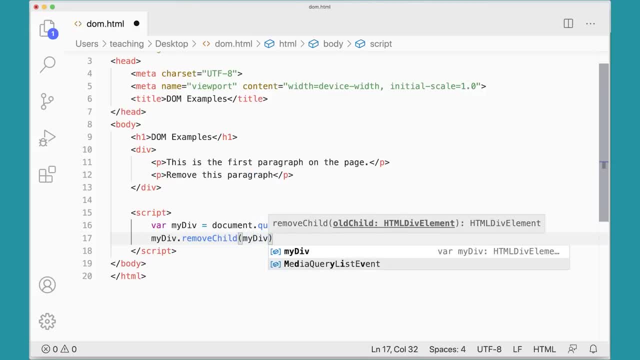 Well, I'm going to say myDivchildren square bracket one. So what that's going to do is it's going to go into myDiv, look at its children, find child number one. Remember, this is child number zero here. That's zero. 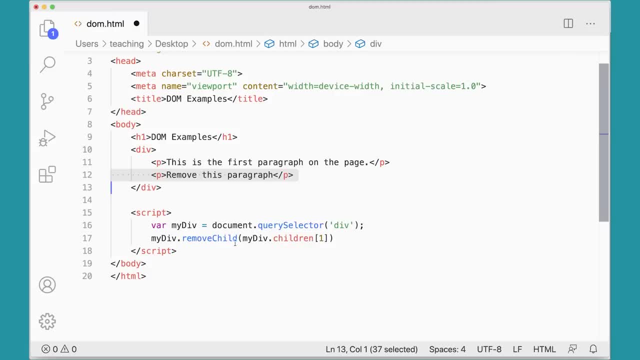 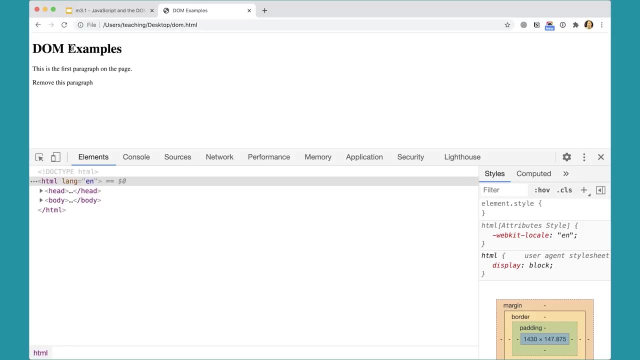 This is one. So that will actually go and remove this second paragraph from this div. Put a semicolon there, Save that And then let's go over to our browser here And you can see I've got the two paragraphs there. When I refresh the page that second one is gone. 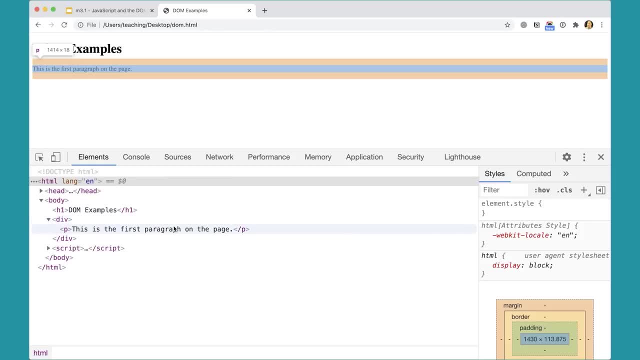 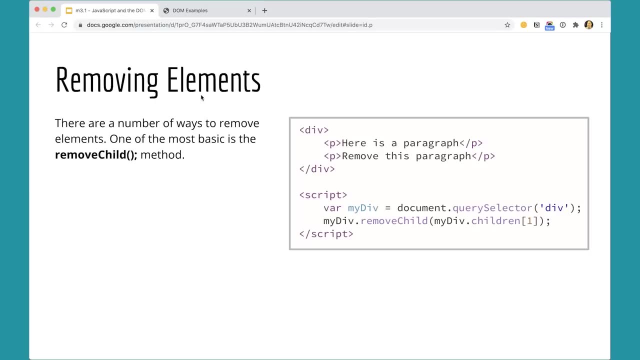 And down here you'll see it's not in here anymore. It's been taken out. JavaScript removed it. So removeChild removing elements using the removeChild method is a really useful tool for removing elements from the page if you need to do that. 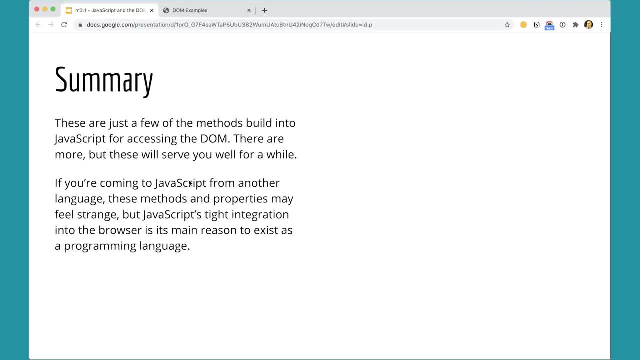 And so here we've seen a lot of different methods that we can use on our web pages to do all kinds of things, And we've talked about this. We've talked about some of the document methods, some of the element methods and some of the element properties. 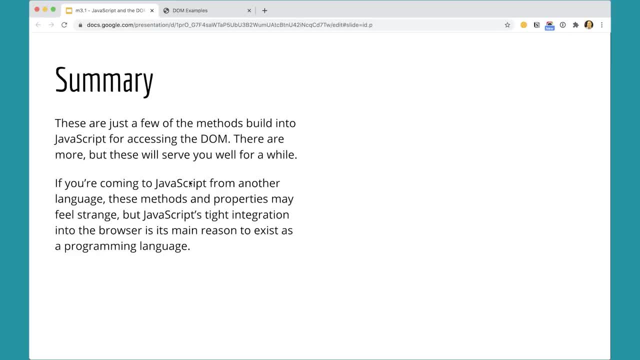 that we can use to go in and affect content on our page. And remember, JavaScript sees the page as this tree of objects, starting with the window and building down from there, And we can traverse that document and find elements on there and then affect them using these different methods and properties. 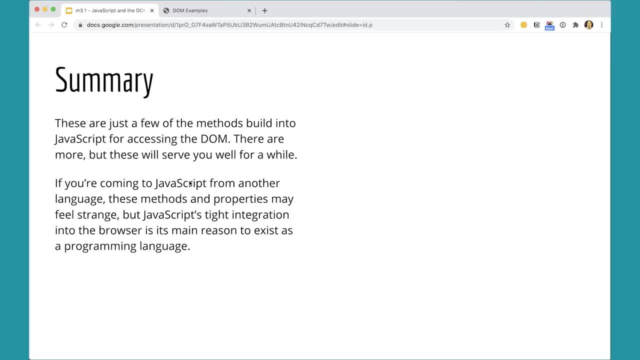 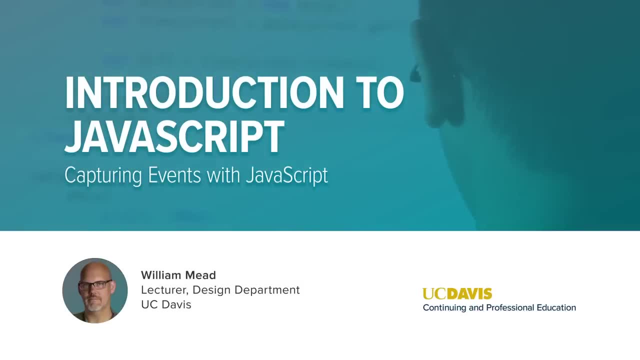 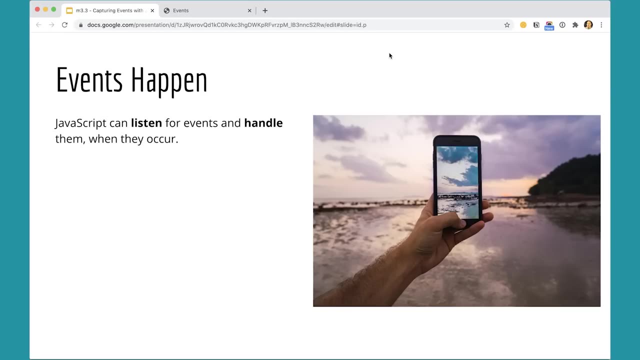 And that's how we're going to create all kinds of interactive elements on our web pages, Capturing events with JavaScript. Events happen, Users will click on something, They'll scroll the page, They'll submit a form. Events happen on web pages. 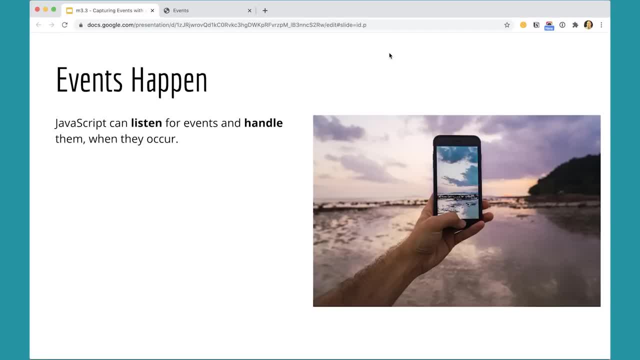 And when events happen, JavaScript can capture them And then they can do something with those events. When we combine this with manipulating the document, like we saw in the previous lesson, this is where a lot of the power of JavaScript really happens, Once we've talked about how to capture events and handle them. 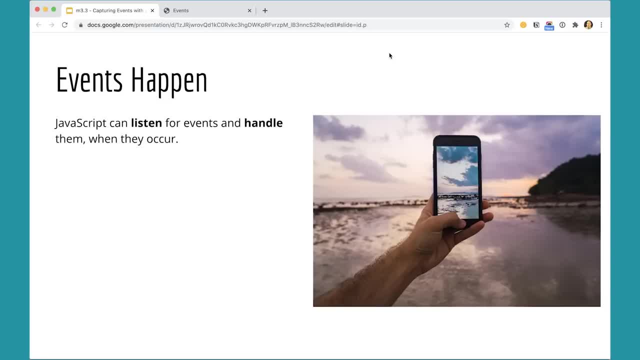 you have all of the basic pieces of the puzzle to make interactive web pages, because we can use our logic flow structures, sequence selection loop, along with our document elements and our document methods and our element methods and properties, to change elements of the page when events happen. 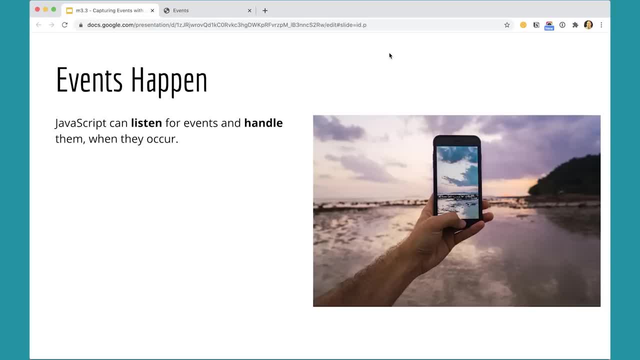 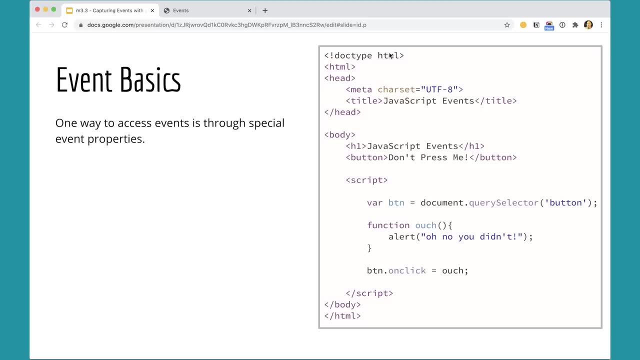 And that's how we can get interactive web pages. Let's take a look at this very basic example Here. I have a web page with a button on it, And when you click the button, it's going to pop up an alert saying that: 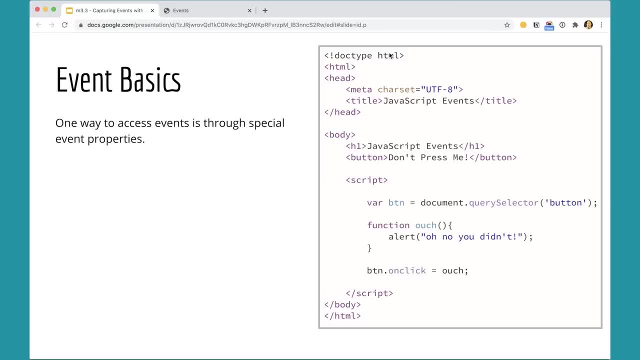 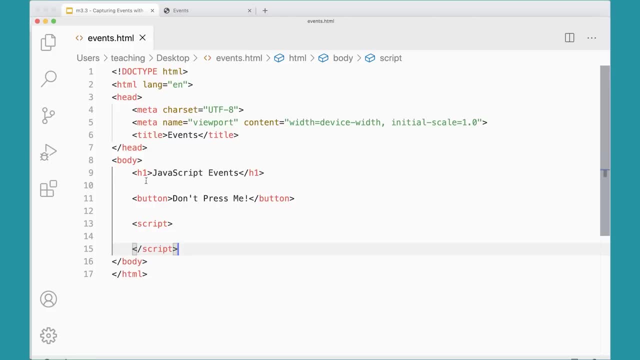 you know you clicked the button, something that shows that you actually clicked the button. So let's go over and do this and try this out Here. you can see I have a web page. I have a button on the web page that says: 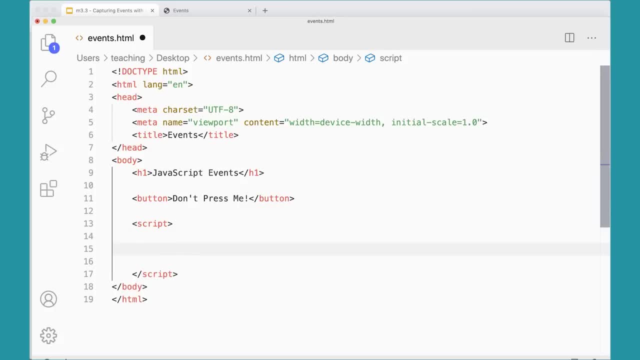 don't press me, And I'm going to grab that button using my document element methods. So I'm going to make a variable for our btn And I'm going to assign it documentquerySelectorButton And then I'll get that button. There's only one button on the page. 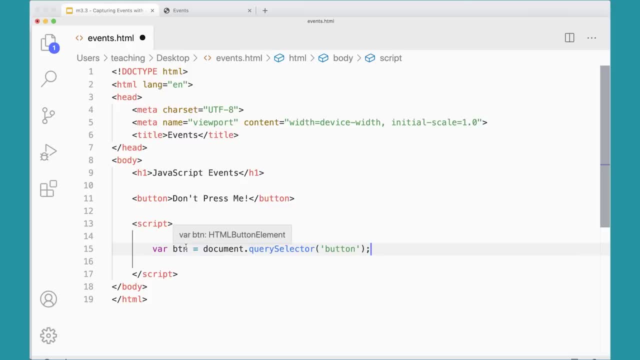 so it's easy to get that one button And it's going to assign it to btn there, And then I'm going to make a function- Remember, we talked about functions. I'm going to make a function called ouch And all that function is going to do is do an alert. 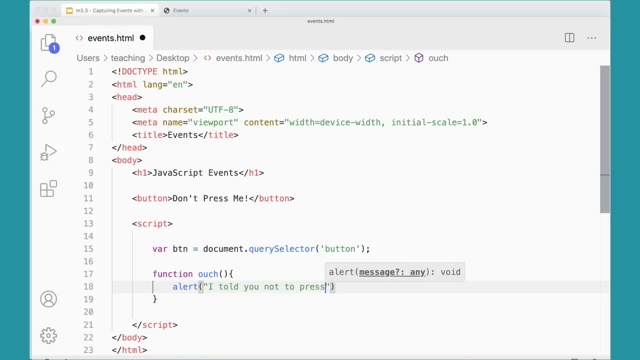 I told you not to, So you press me. You can put whatever you want in there, That's fine. And then I'm going to say, okay, btnonClick, Run this function. Ouch, So that's going to actually run a function. 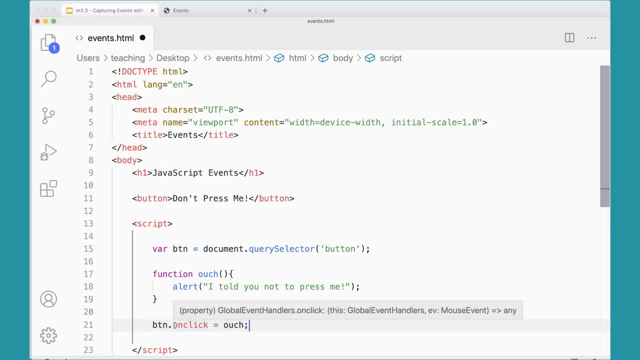 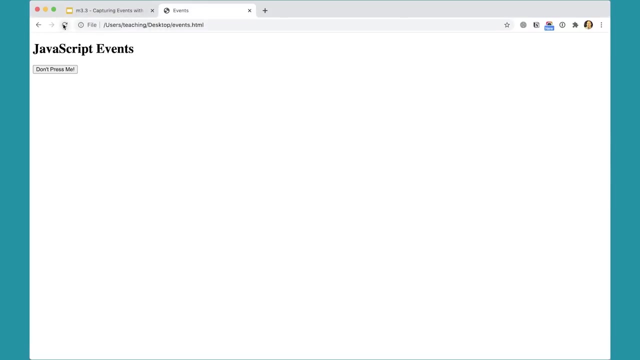 using on the button, And we're using here a special property that will capture the click event. So let's do that really quickly, Let's see if this works. If I come over here and refresh the page, if I click, don't press me. 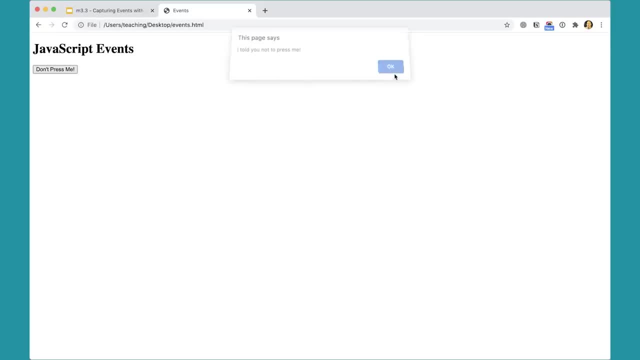 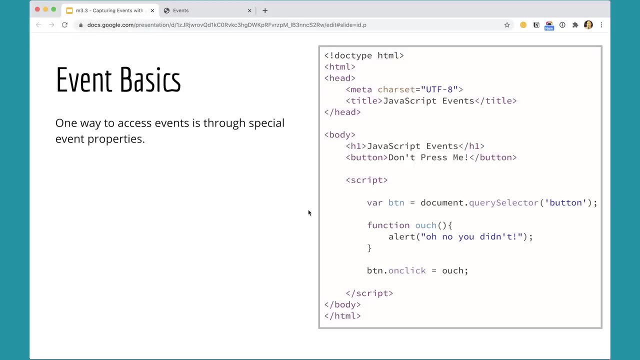 I get an alert that says I told you not to press me, So I'm capturing that event of the clicking of the button. And the way I'm capturing that event is with the onClick property. One thing to notice is that I define this function. 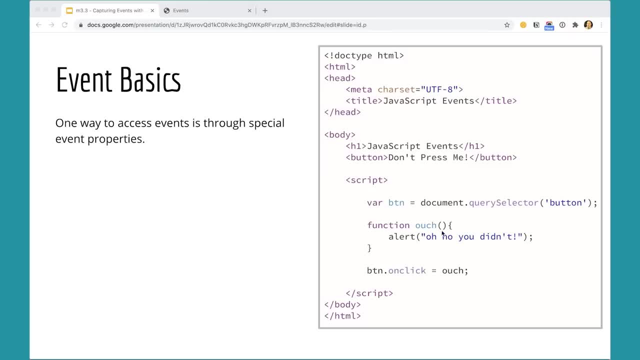 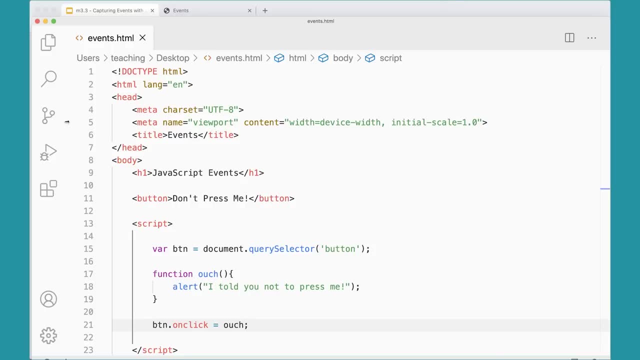 And when I assign the function to that property, notice I don't put the parentheses at the end here. If I did, then that function would run right away. It would run immediately. So if I put parentheses here, you will notice that it's not going to wait for me to click. 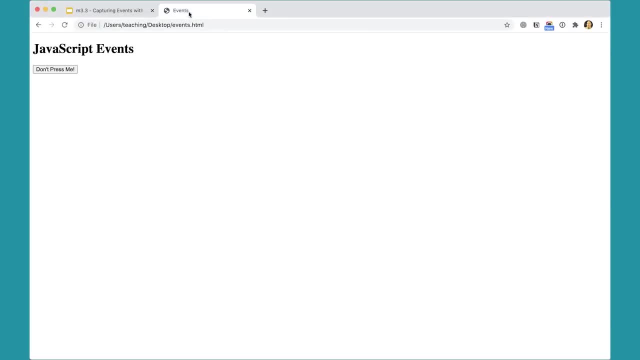 Instead, at the end it's going to run right away. So if I come over here and refresh this page, you'll see I get the alert without even clicking the button. So when I use the event property with the function that I've created this way, 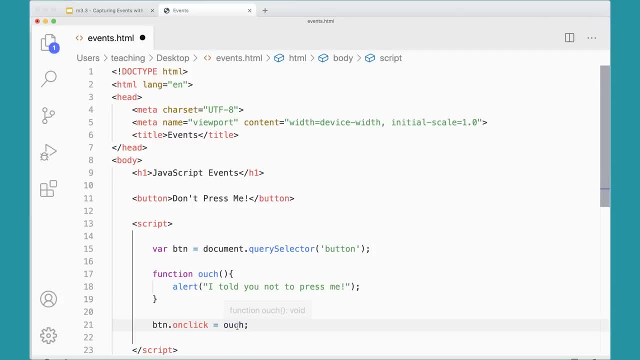 I do not add the parentheses for the function there. I just reference that function by name, Ouch, And it will then run that function when the event runs. Now you don't have to define a function here. We can actually just use an anonymous function here. 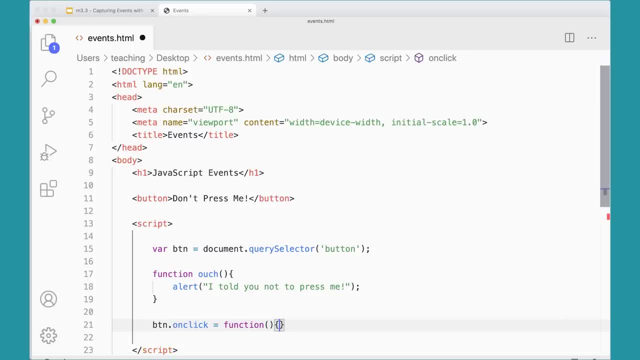 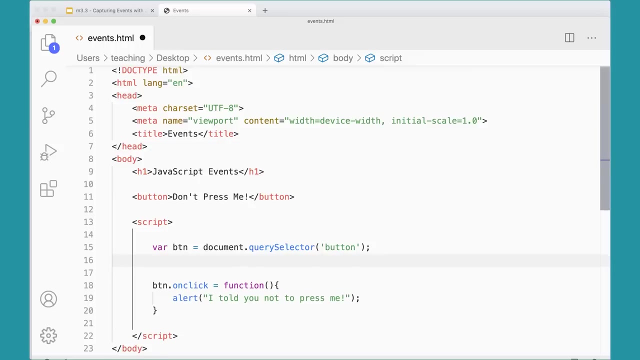 So I could say: function parentheses, curly braces and just stick the alert in here and get rid of this altogether. And frequently when you're using something like this, you're only going to run this on this particular button in this circumstance, So there's not really a reason to create. 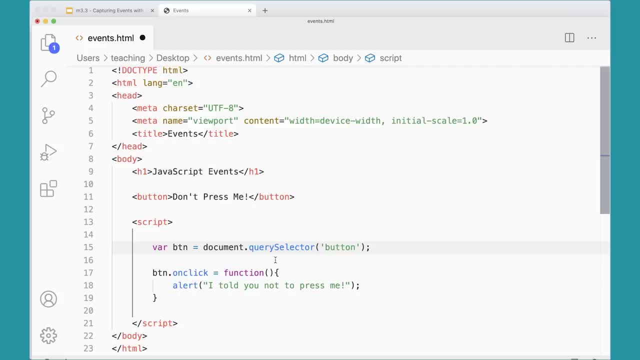 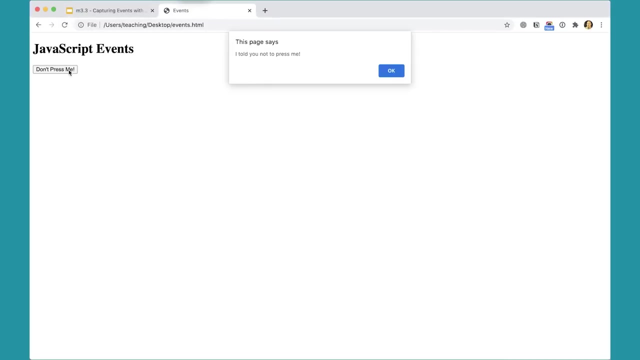 a named function that you could use over and over again in this case, if you're only going to run this in this one case here. But let's see if this works. Refresh, Don't press me, And I'm getting the alert So I can use the anonymous function to do that. 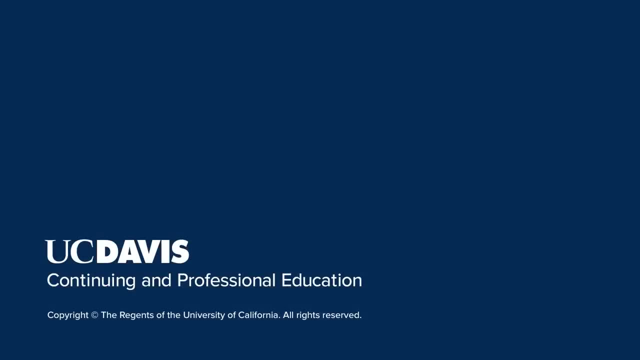 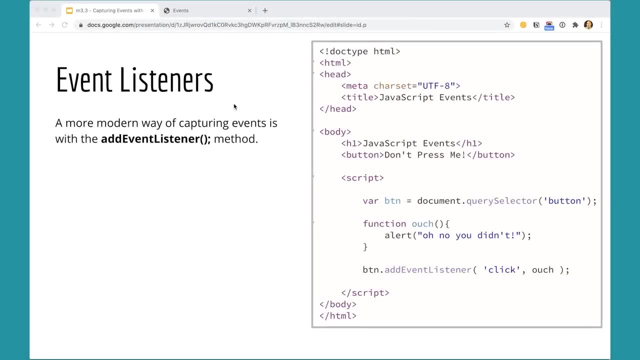 Let's see if this works. The onClick event property is useful, but a more frequent method that you'll see of capturing events is using the addEventListener method. This is a great way of capturing events, because you can capture all kinds of events with the addEventListener method. 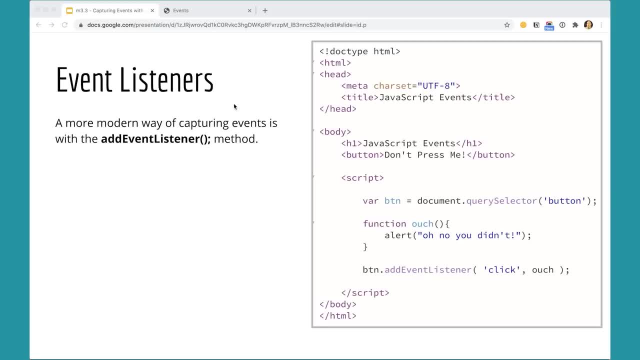 You can even tell it what type of event you want it to capture. And what's really great about it is you can actually put multiple event listeners on one element, whereas with the event property you can only put one. You can only be listening for one thing at a time. 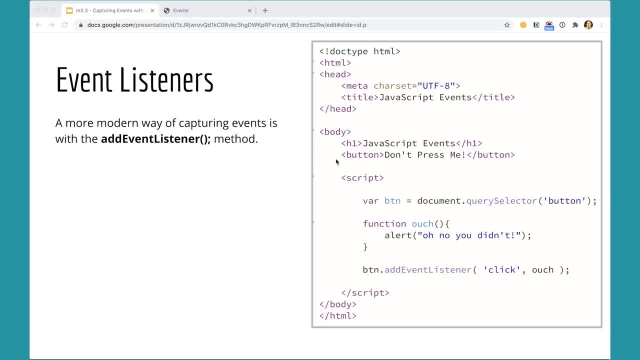 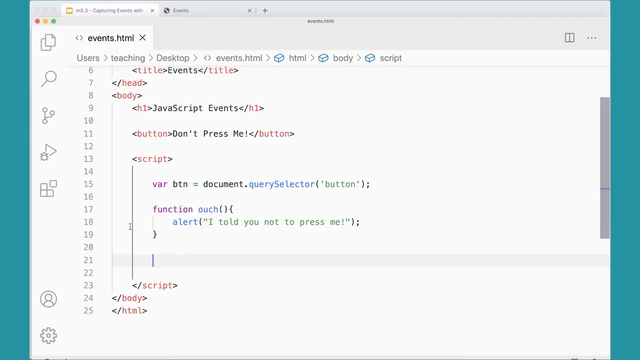 So here I'm going to go back to our version with the function ouch and the alert in there, And then we'll use the addEventListener instead. So let's give that a try really quickly over here. So instead of using the onClick event for button btn. 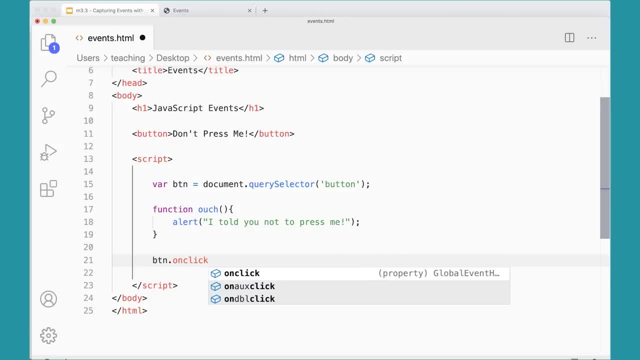 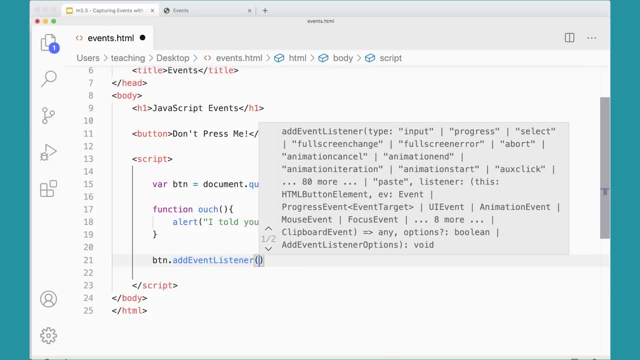 instead of onClick that event property, I'm going to use the addEventListener method And notice the difference between the two. The onClick property is a property because it's onClick and then an equal sign in what you're assigning to it With addEventListener. 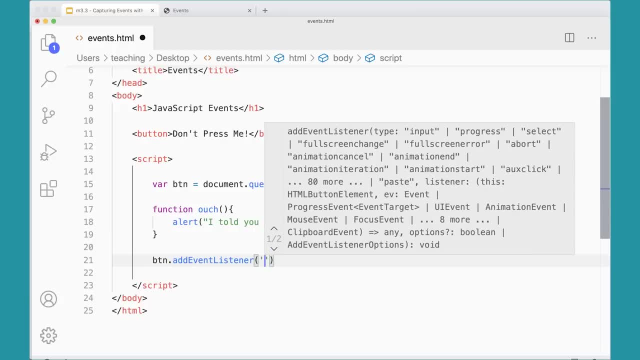 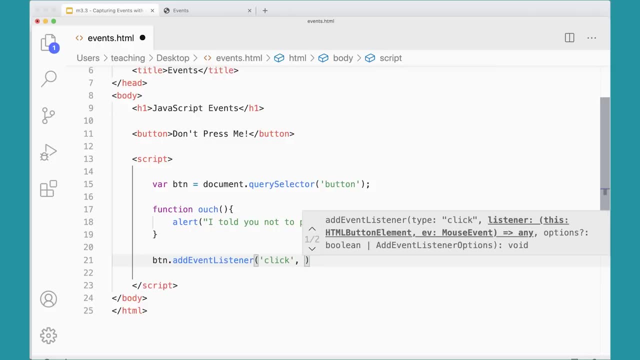 it's a method, because it's got parentheses And we're going to pass in a click That's the event we're listening for And then we're going to pass in the function that we're going to run when that event happens, And this is a very much more modern way of doing things. 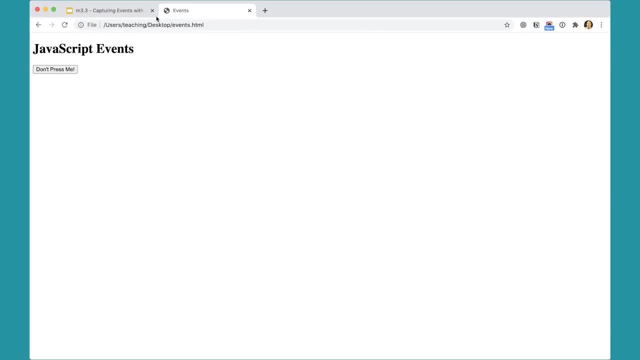 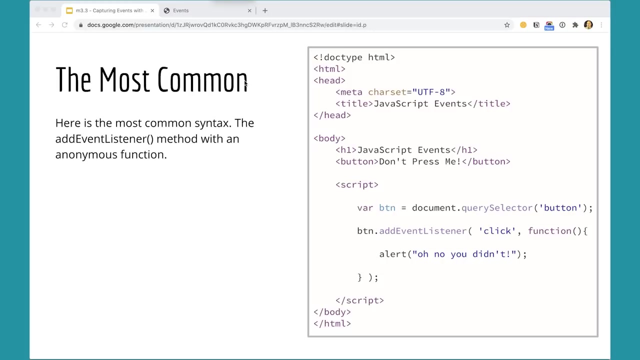 It's using the addEventListener method here, So let's see if that works. And sure enough, it works just the same as before. The most common syntax is to use the addEventListener with an anonymous function, So it kind of combines the two that we looked at before. 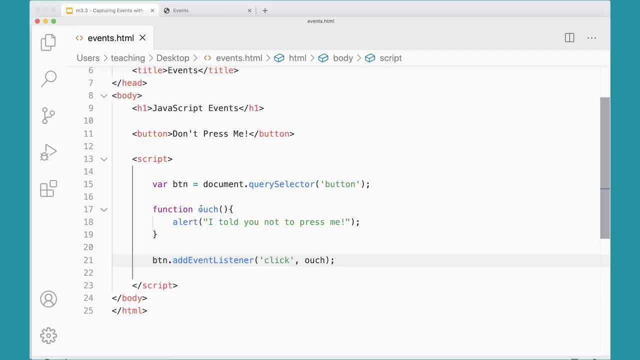 So let's take a look at that instead. So down here, instead of running the function here, ouch, we're going to put in an anonymous function function with its parentheses and curly lines, And this function is going to run when the click happens. 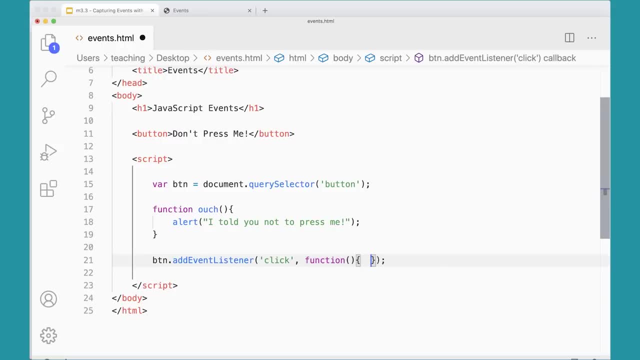 And in here inside the curly braces, is what it's going to do. So we're going to put in there the alert, Stick that in there, And then we don't need this function at all. So you can see that we're running this. 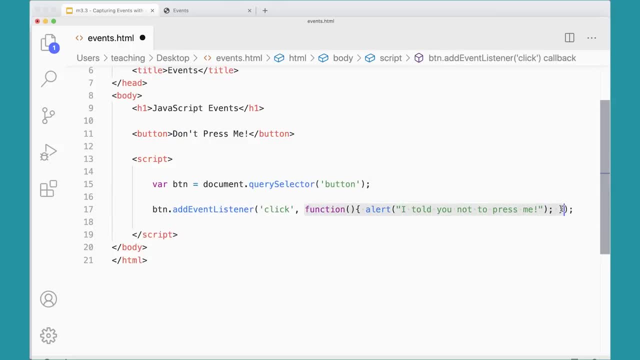 This function starts here, It ends over there. We're going to run that function, that anonymous function. And again, we use an anonymous function because unless you're going to be running this alert on lots of buttons, in which case then it does make sense to pull it out. 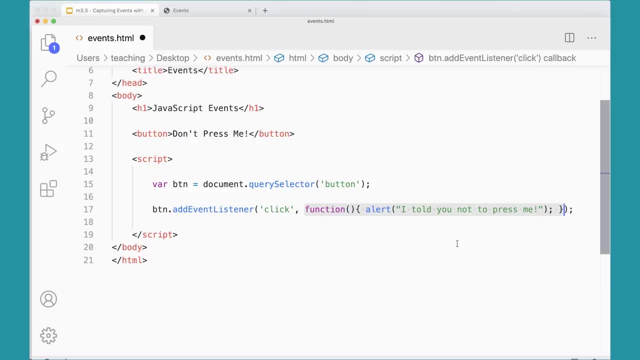 and turn it into a separate function. But unless you're going to do that, you're probably only going to use it within the context of this particular button, And in that case an anonymous function is more appropriate. So we can save that. 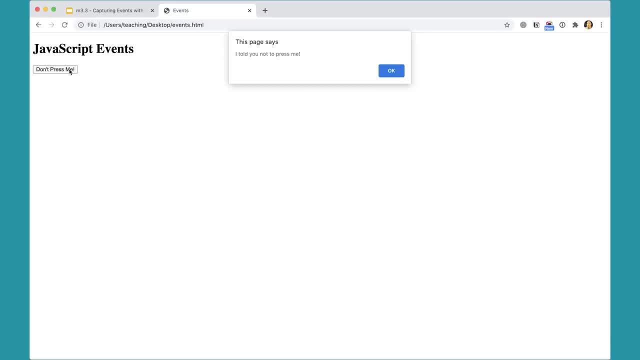 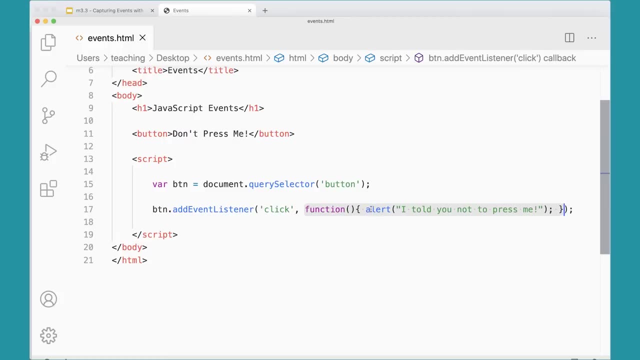 I'm going to come back and let's just test it one more time. Refresh the page, Don't press me, and I get my alert. So that works great. Now, this syntax, this line is getting kind of long here. Usually you would break it after the curly brace. 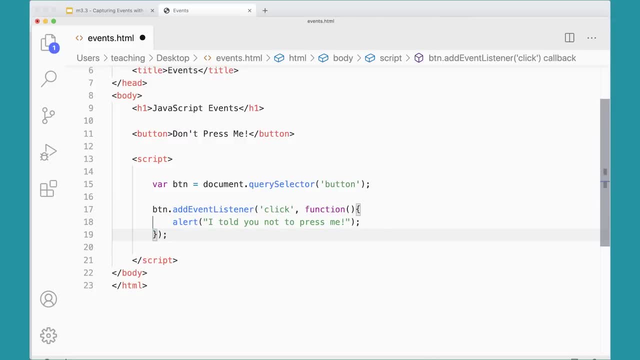 And then this curly brace can come down here. Notice when I type this. One last thing I want to show you before we go. I'm going to do it again. Notice when I type it. I type it from the outside in, So I type my function. 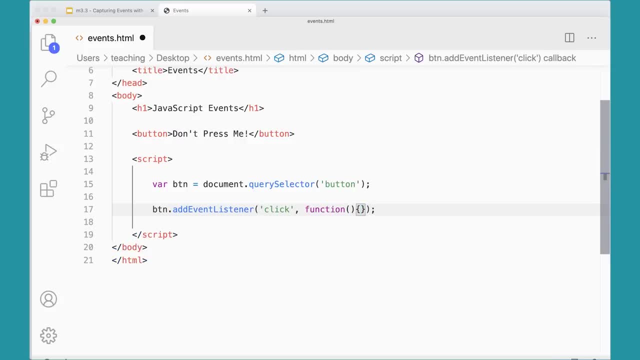 with the parentheses and the curly braces, And then I come in here and I add my alert or whatever I want to have happen inside this function here, Because with doing this you're going to end up with a bunch of extra punctuation here And it's really easy to get confused. 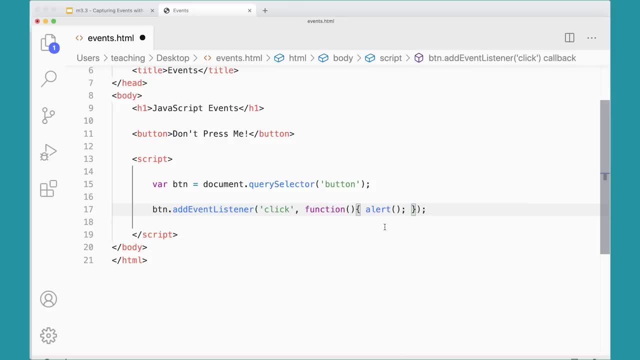 And if you lose a curly brace or a parentheses or a semicolon or something else, it's really hard. Those problems are some of the harder ones to track down And you'll have fewer problems, You'll be less frustrated if you do it this way. 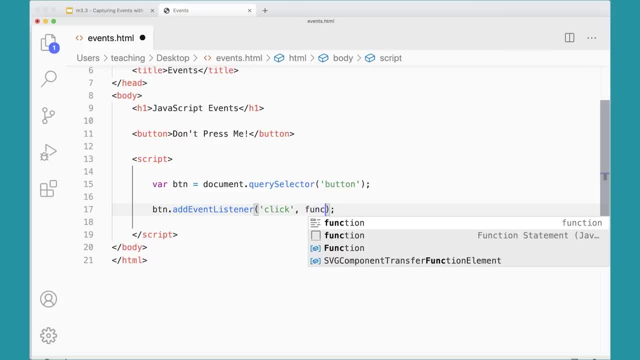 where you always type from the outside in. So when I add a function, I type its parentheses and curly braces and then go inside and put in what I want to put in here. Okay, So that will really help you with making sure that your syntax is clean. 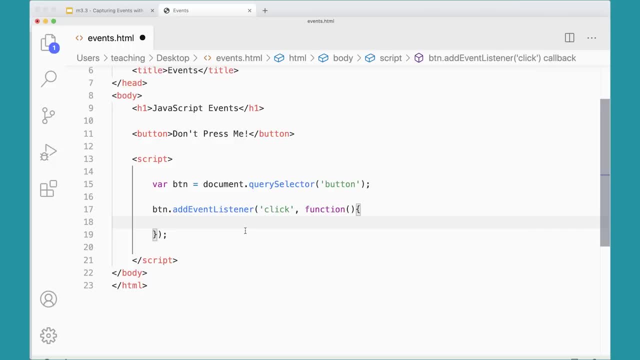 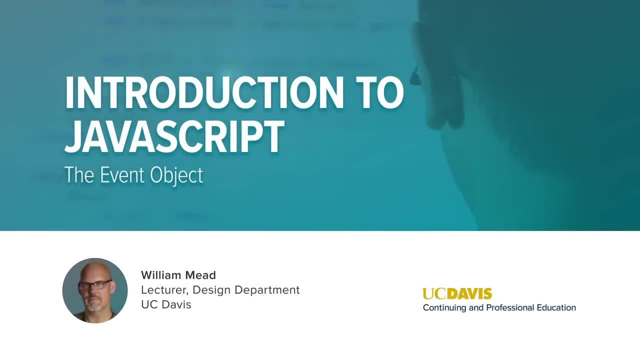 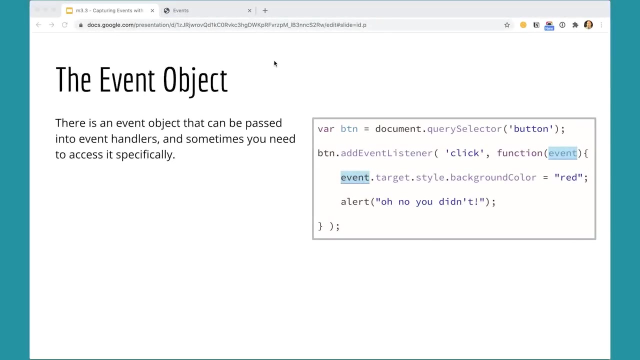 and that it's going to have fewer errors. The next thing to look at is the event object. The event object can be passed into the function that runs when an event listener happens, And it's a very useful object to have access to. Let's take a look and see what it does. 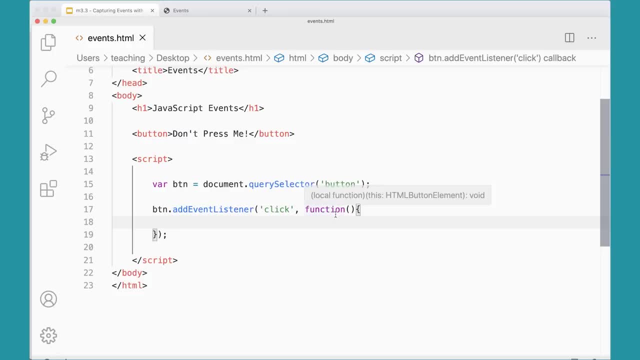 So over here I'm, in my event, listener here and I have this function here And I could still do my alert here. Alert, I told you not to press me or whatever I want to put in there, But I can also put in. 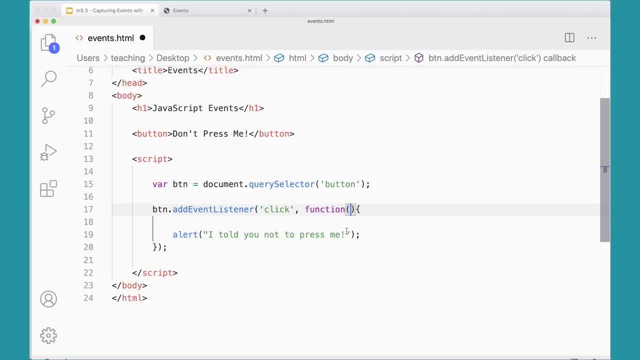 I can also put in, I can pass in the event object And sometimes it comes in looking like this: This is just a variable that represents this event object And I can pass that in and I can do event dot target. The event target will say: 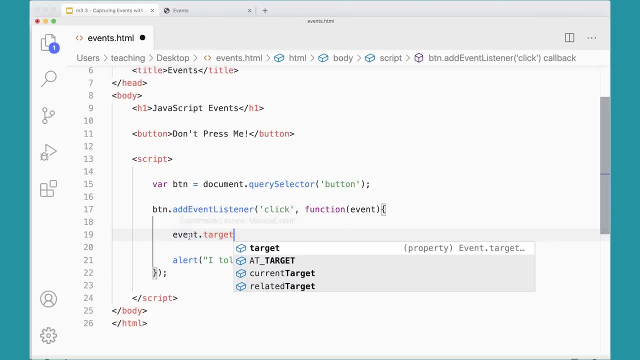 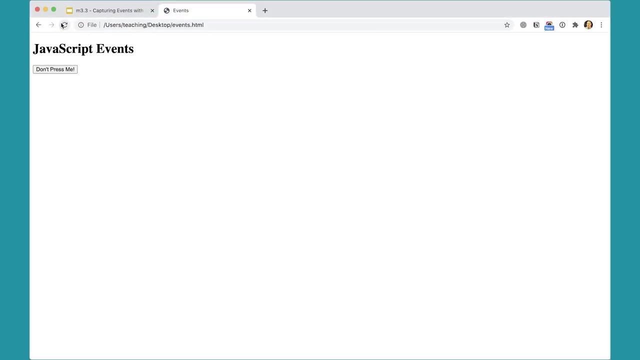 what is the thing that triggered this event? Event target dot. target Style dot. background color equals red, Something like that. Let's see what this does. If I come over and run this, Refresh my page, Don't press me. It does that and sets the background of the button to red. 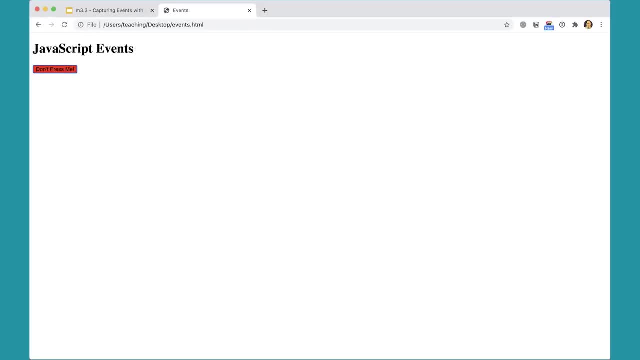 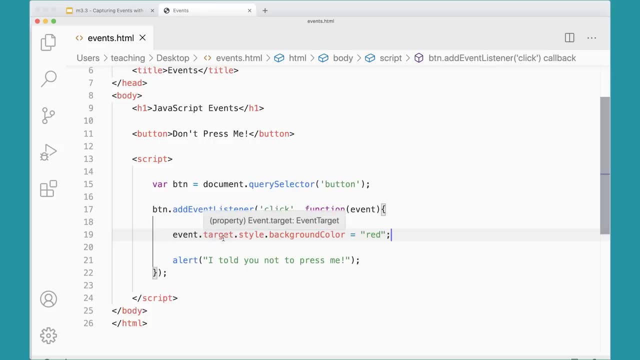 which is very interesting there. So what's going on here is we can use the event object and the event target to actually know which element was triggering this event, And then we can do something with that event target, And that's. this is often very useful. 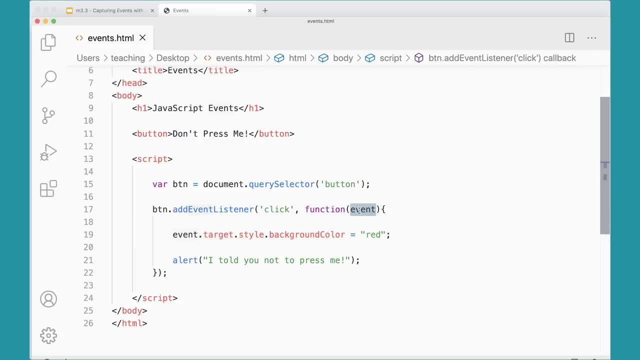 Now, this thing is just a variable. Sometimes you will see this: If you look around on Stack Overflow, you'll see people pass it in as EBT, In which case this would be EBT, Or sometimes you'll see just E. 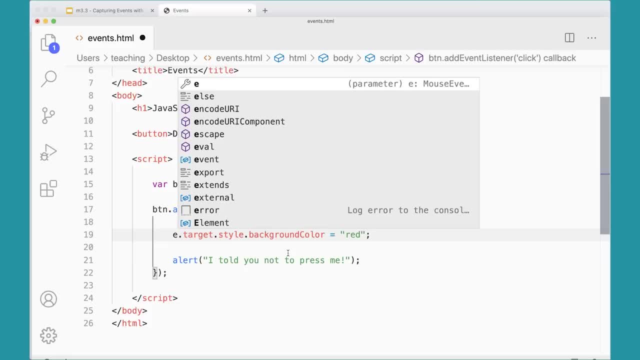 E, That's fine. It's kind of nice and short. You could call it whatever you want It represents. call it chickens if you want to. It doesn't make sense to call it chickens. Chickens target style doesn't really make any sense. 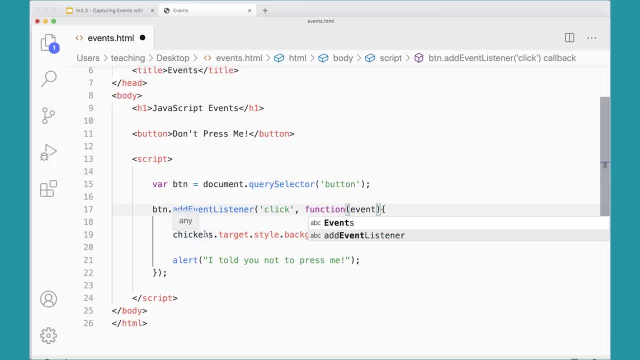 So usually event makes sense Or EBT or E- But you'll see it represented in different ways. if you look around on the web, If you look at Stack Overflow, you'll see people putting in different values for that event. But the thing that we're passing in here 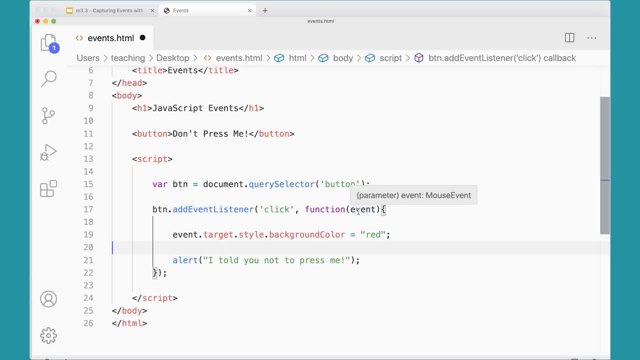 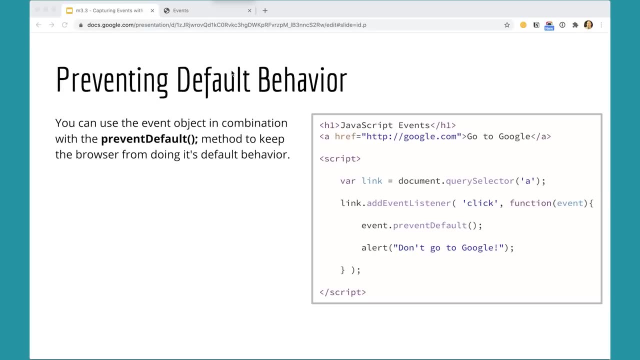 is the event object. Just to be really clear about that. One of the ways the event object is used most frequently is to prevent default behavior, And this is especially true when we're working with forms and with the submission of forms. We want to prevent the default submission of the form. 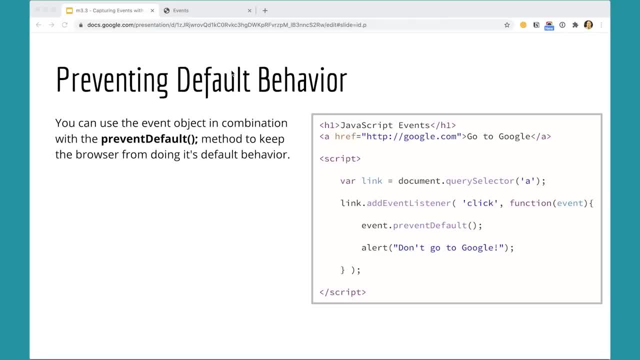 so that we can do something with that form data before it's submitted, And so we'll use that frequently. But let's just take a look at a really simple example of this here. So if I go over to my code editor over here, 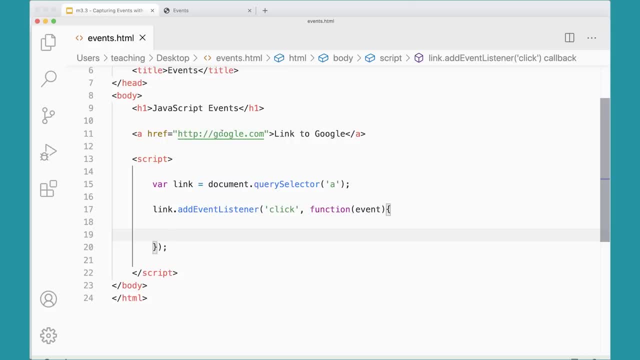 I have just a link to Google here, Just a normal anchor tag with an href going to Google, And down here I have a variable link. document query selector A is going to go into my document and find the first anchor tag that it finds. 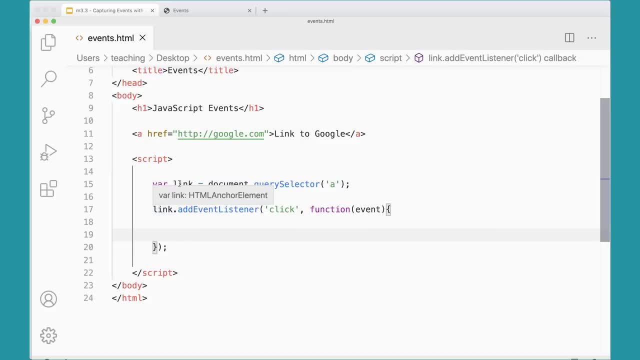 which is the only one on the page, And then I've got attached to that link. add event listener when you click passing the event And we'll use the event object in combination with event prevent default, the prevent default method, to keep that, keep that default method from happening. 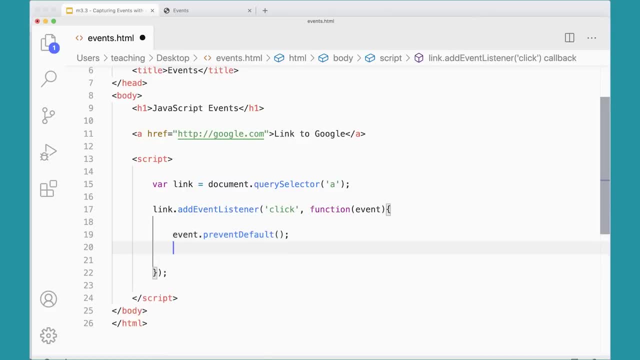 The default action from happening. In this case we won't go to Google, So I could do alert. Sorry, No Google for you, Something like that or whatever you like. So now, if I test this page and I come over to my events page and refresh here, 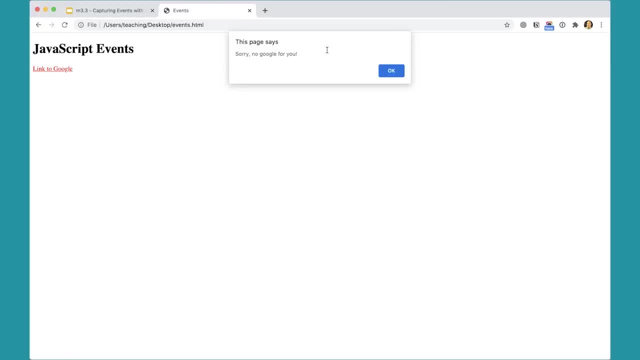 I now have a link to Google And when I click it I get sorry, no Google for you And the page does not go to Google. but it's really the event prevent default. It's keeping it from going to Google. If I were to come back. 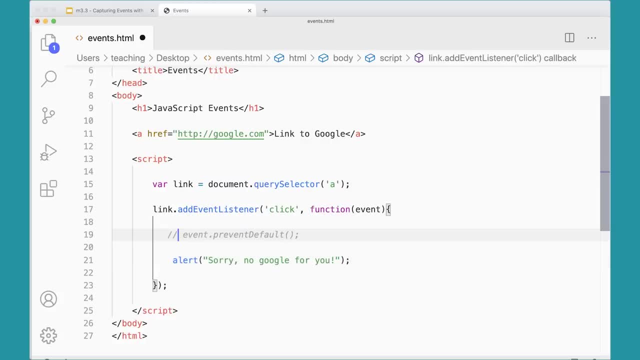 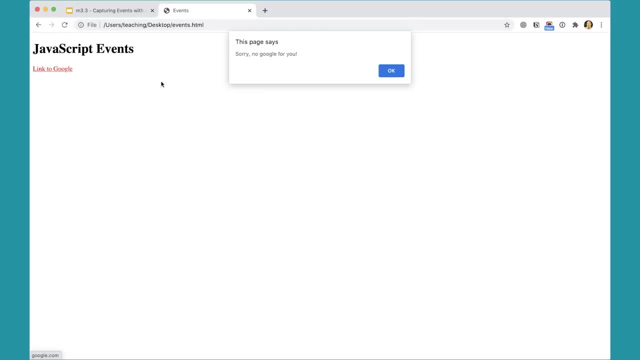 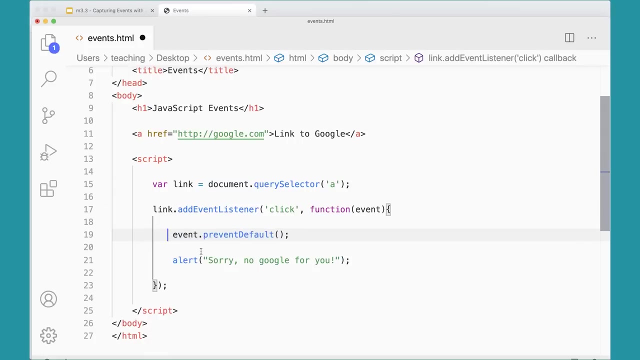 and comment this line out here, you'll see what we get over here. If I refresh, I get the sorry no Google for you, but then it'll actually go to Google. Okay, Because the event prevent default is needed in order to keep that default event from happening. 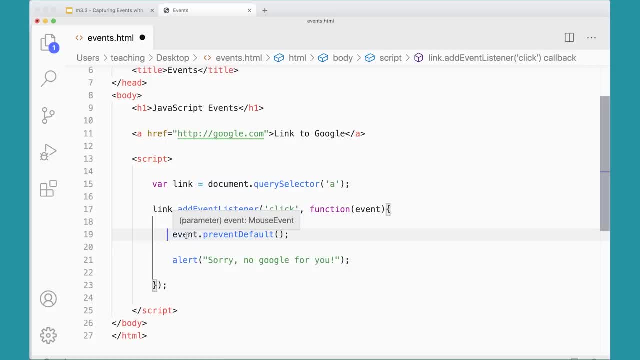 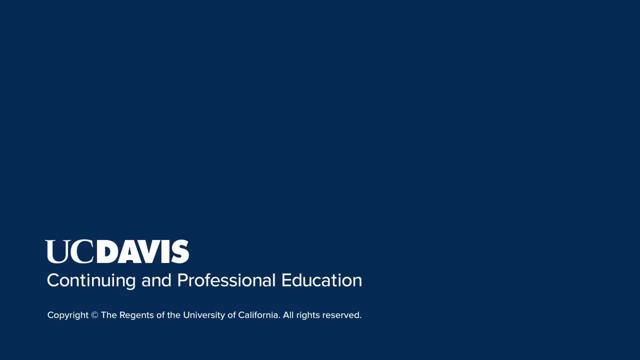 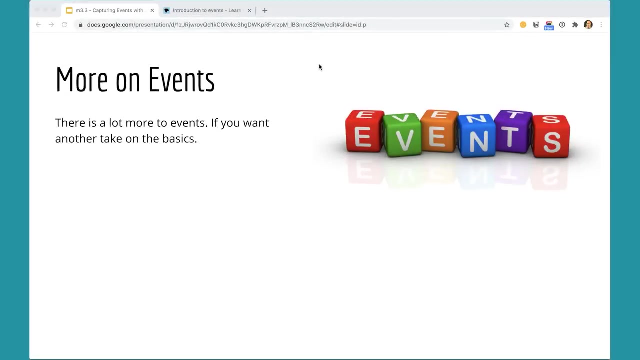 So this is another. this is a particularly useful function that we can use with the event. object is prevent default, And we'll be using that frequently in a number of our projects. There's a lot more on events And if you want another, take on the basics. 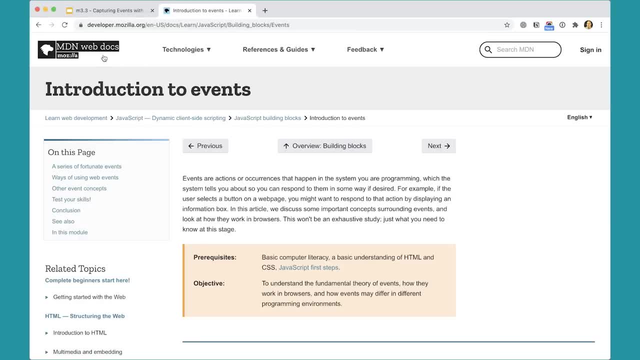 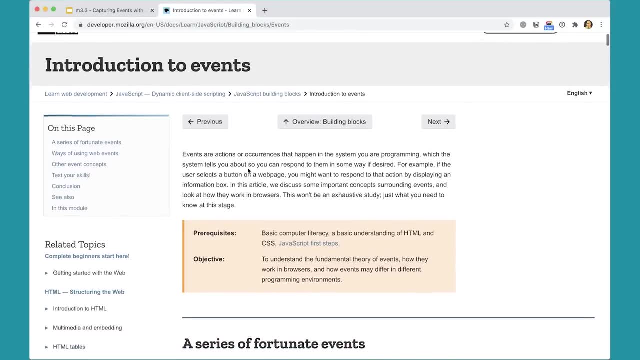 you could go to this MDN web docs page on introduction to events. I'll put the link in with the lesson so you can click it and look through this page. And this page gives you a very thorough overview of events and the way they work in JavaScript. 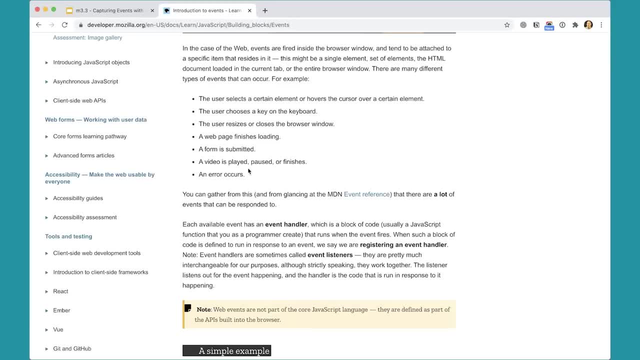 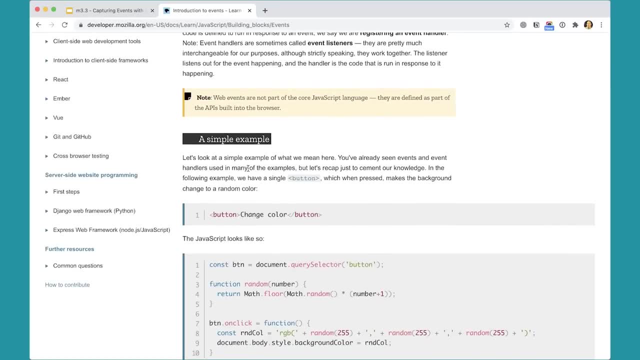 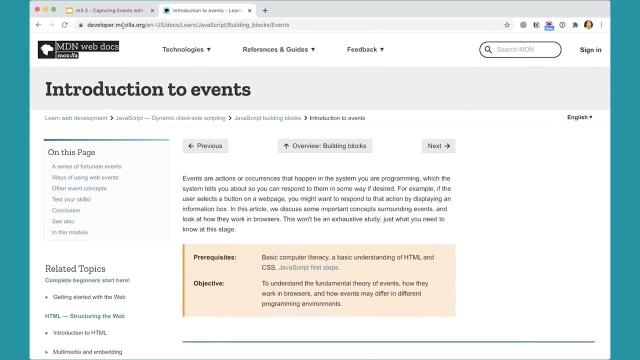 And some of the more advanced things that they get into, like bubbling and propagation and all this kind of stuff we'll look at later in the course, But this will give you a thorough introduction to events in JavaScript here as well. What we're going to do next. 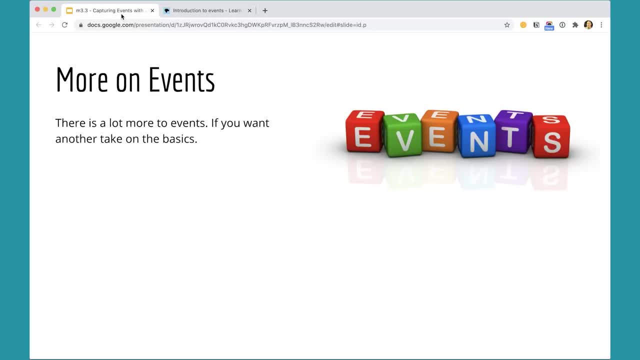 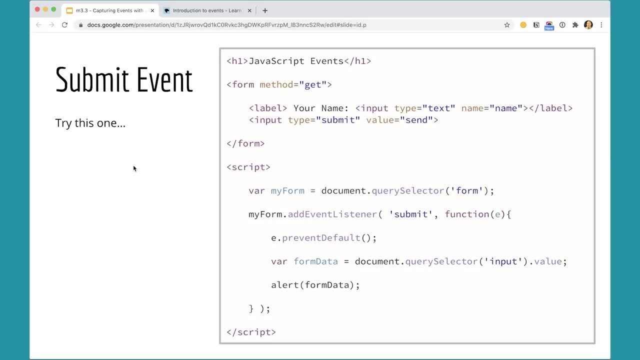 is actually capture some different types of events and see what we can do with them in JavaScript. So the first one we'll look at is the submission of a form. So let's take a look at this example really quickly in the code over here. 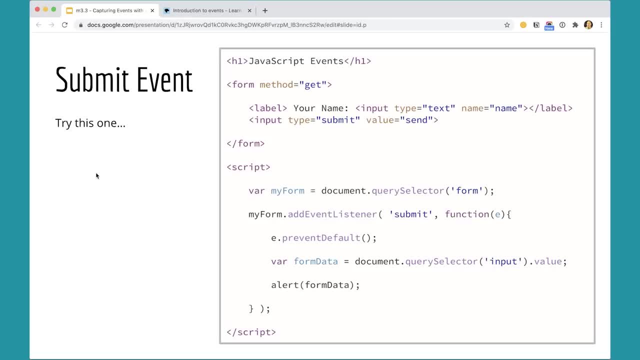 And I recommend that you actually type these out and save them, because they're going to be really helpful to come back to when you do the event challenges coming up or for some of our other projects. it'll be helpful for you to have these little small scripts. 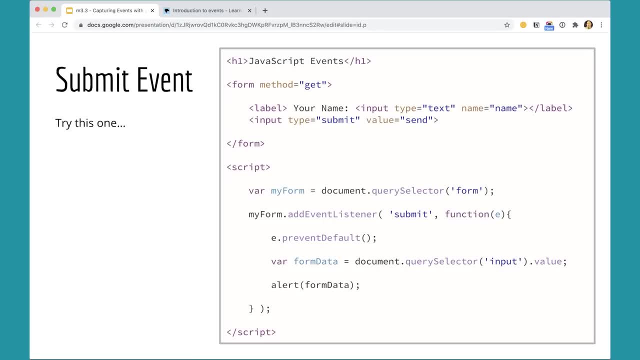 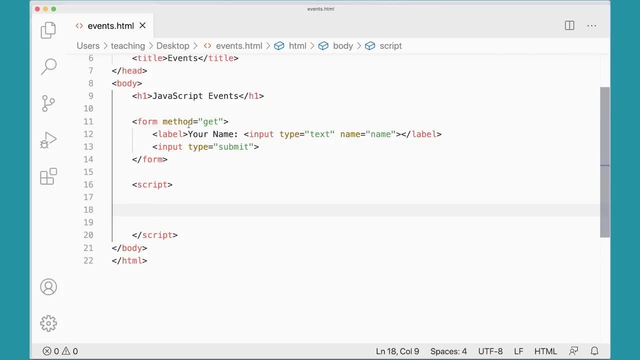 to reference to see how to do things later. So I recommend typing them out. So here I am, over here. I've got a form on my page here. It's set to method get. We'll see why in a few minutes here. 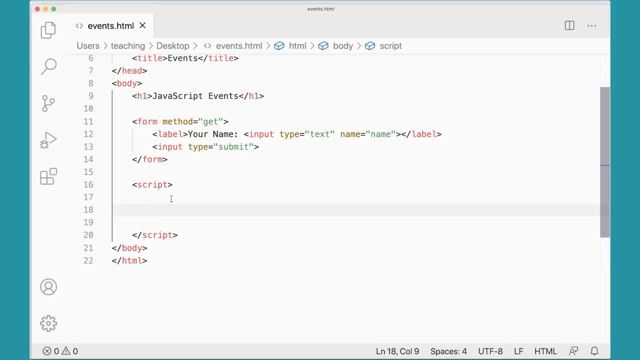 And down here I'm going to just get my form and stick it into a variable r, my form Documents. I'm going to use my document query selector method to get the form. There's only one on the page, so I don't have to do anything special there. 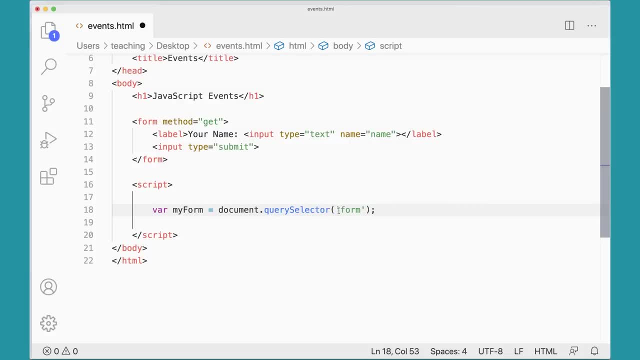 If I had multiple forms I could give it an ID And then I could get it by the ID, And that would be fine too. But since I only have one, that's kind of nice and easy And that's great. That gets me my form. 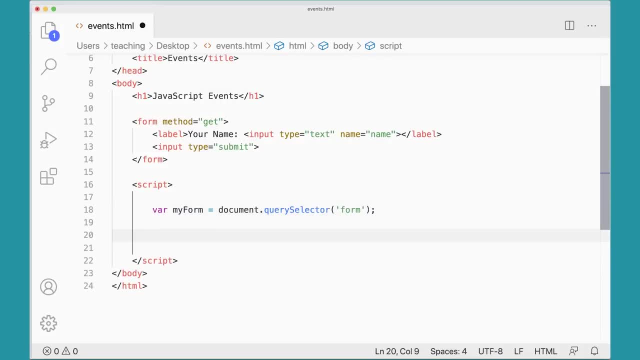 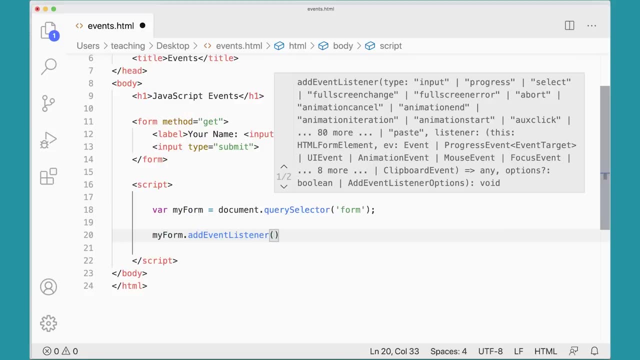 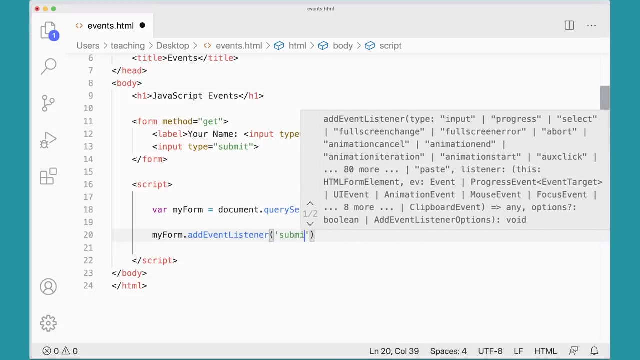 And then I'm going to put an event listener on that form, My form dot. add event listener. And the event that I'm going to look for this time is the submission of the form Submit, If I can spell it right. Before we looked for a click. 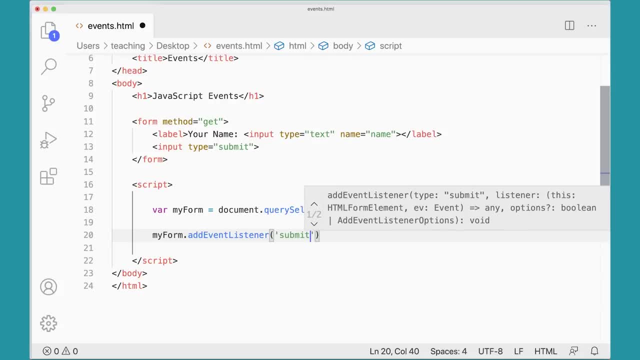 And often we want to capture clicking of things, But in this case we want to capture the submission of the form. So I'm going to look for a submit And then I'm going to run a function when the form is submitted. I'm going to put an extra space here to make it really clear. 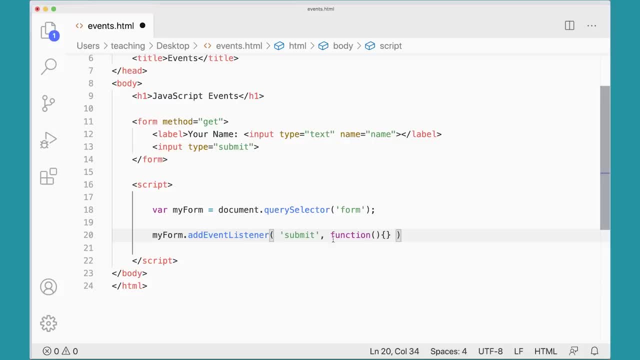 that these things are in here. So we're looking for a submit, And then we're going to run a function, Put a semicolon there, And then what I'm going to do is going to go inside the function here. Now, the very first thing I'm going to do 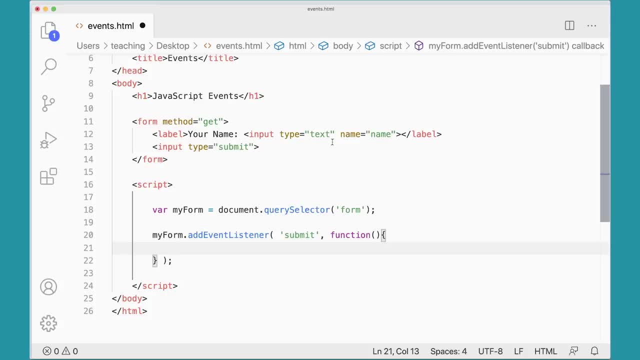 is, I want to stop the normal submitting of the form. I want to do something other than that, So I'm going to pass in my event object here. In this case, I'm just going to use E as a shortcut And then down here I can do: E dot, prevent default. 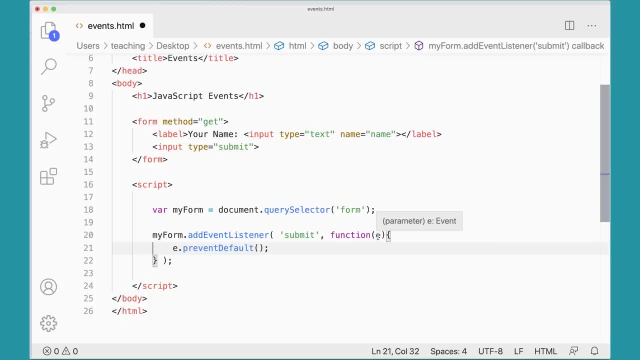 Now this could be event or EVT. Sometimes E is confused with error, So maybe being a little bit more explicit is better, But this should still work just fine. OK, So I'm going to prevent the default submission of the form Great. 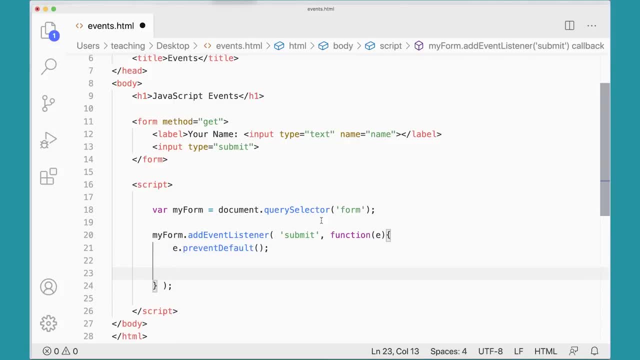 So we got that working. Next, I'm going to actually get the value that somebody types in this field up here And I'm just going to alert it back to it. It's not very exciting, But it gives me kind of an idea of something I can do. 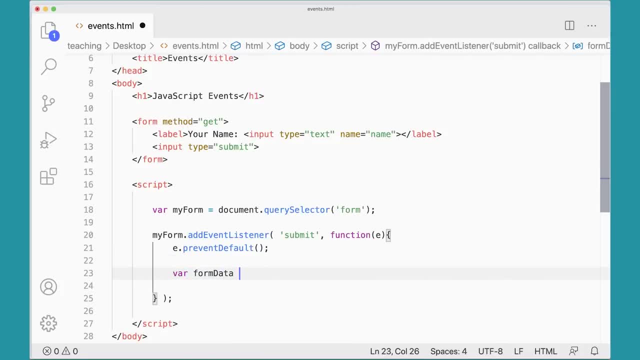 So I'm going to do var form data equals document dot query selector And I'm going to just do input In this case, because this will actually go and find the first input. it's going to find this input here And really what I want is the dot value. 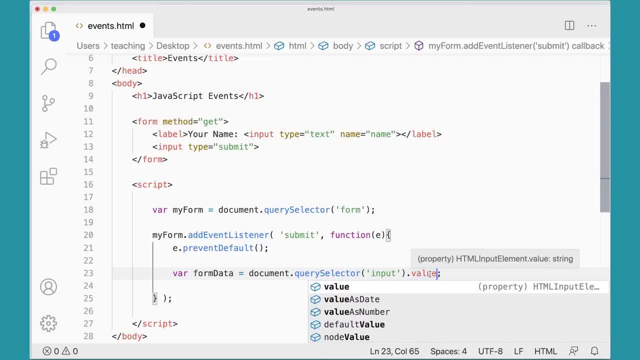 OK, So I want to get that property, the value property of this input, here. Now, if you're not familiar with HTML or not very familiar with it, I can add a value here: value equals bill- And that will come up by default. 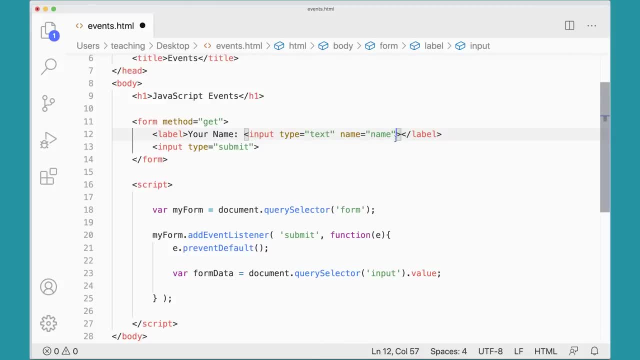 But if somebody types a value into the field, then that default value would be replaced with whatever they type into the field. So I'm getting that value property. Since I'm not adding the property there explicitly, it'll be whatever somebody types into the field. 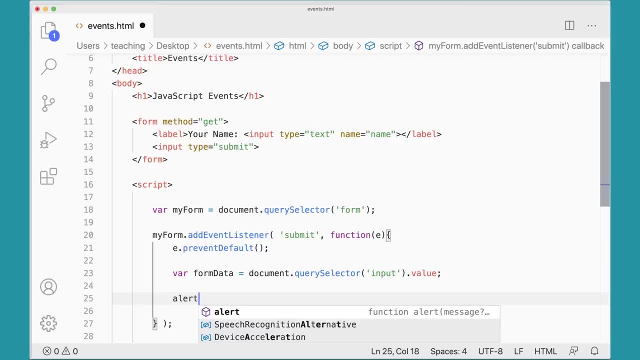 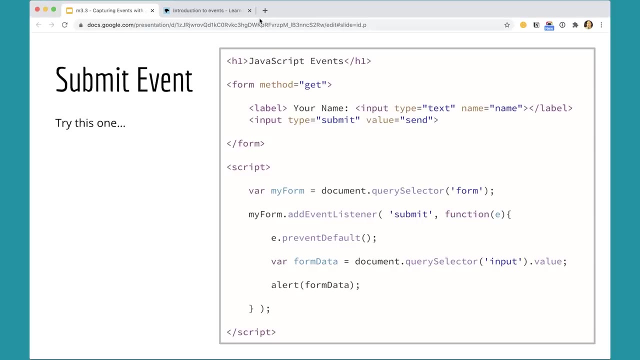 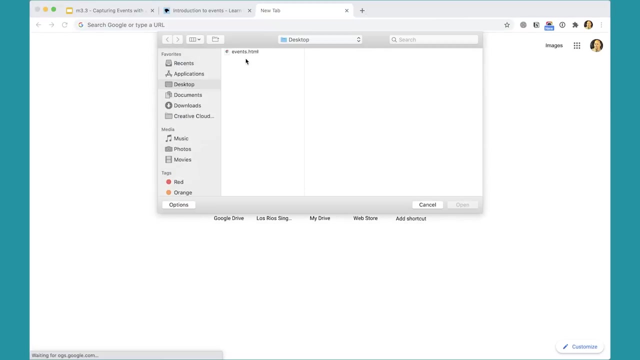 OK, So then I can just alert out alert form data. And now, if we go try this, I need to open my file again. Events Open- Here it is, And if I type something in here bill and submit, you'll see it says bill. 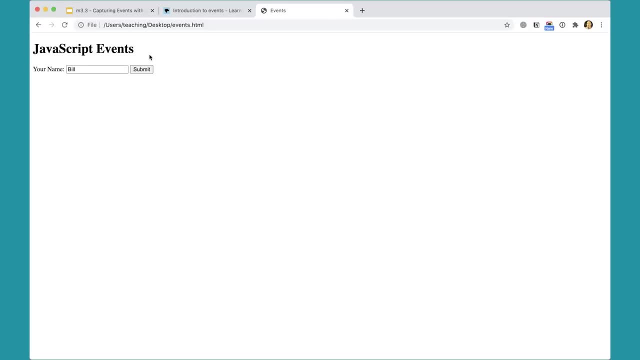 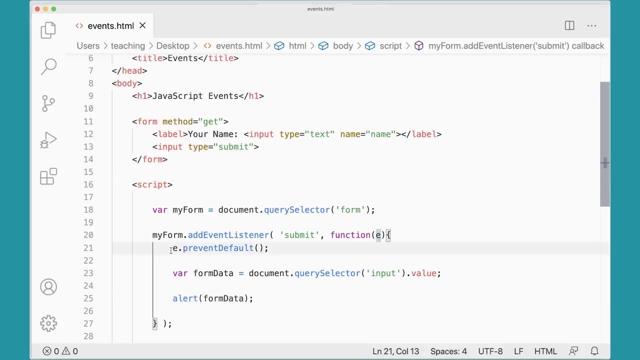 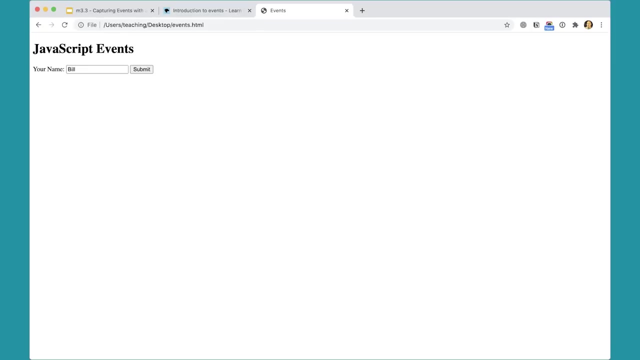 And the form data is not processed. The prevent default has kept this from happening. So if I comment this out for a second, watch what happens here. Refresh this. If I type bill again And now if I click submit, you'll notice it does that. 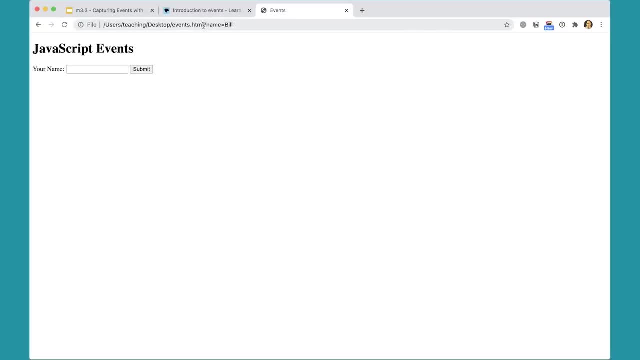 But then it actually processes the form And I can see that up here because I used the get variable. I used the get method. It's actually putting the value that I typed into that field up in the URL By default: a form. 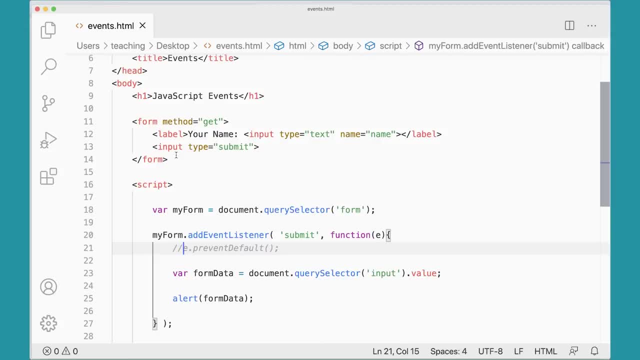 a form element when you submit it, the default behavior is that it will go to whatever you set the action here. If I had an action equals processorphp- some other file that's going to process the data- it would go to that page or it would try to. 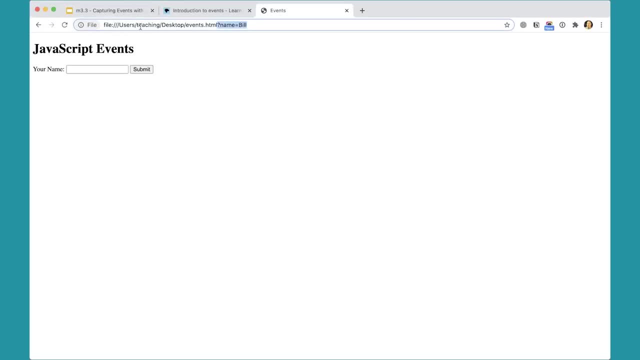 In this case it won't be able to because that page doesn't exist. OK, If I do bill submit, it's going to do that, And then it's going to go look for processorphp, But that page doesn't exist. 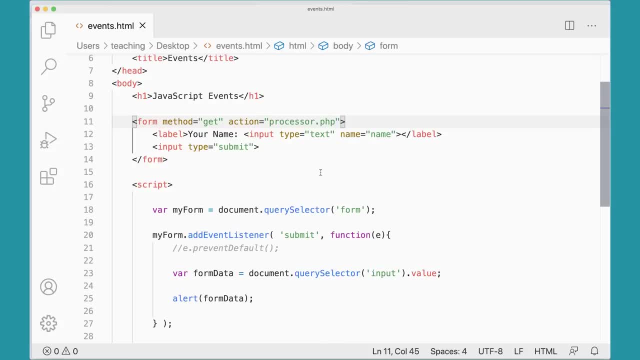 So it either tries to go there or it just refreshes. If I don't put an action attribute up here, it will just refresh this page, And often I don't want to refresh the page. I want to use JavaScript to capture this data and do something with it. 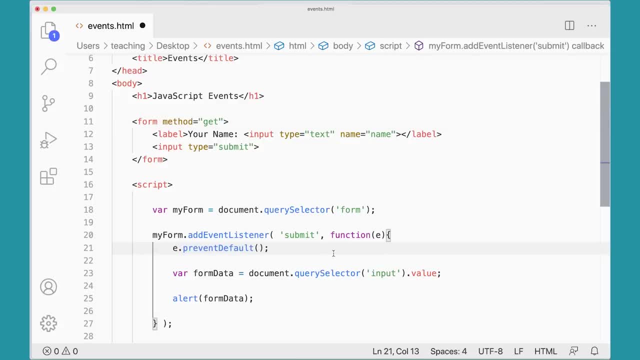 So that's why I'm doing prevent default down here And I'm passing in this event. And E again is a little bit unclear. Maybe use EBT instead if you want to keep it short, And that will pass in that event. object: and prevent the default behavior. 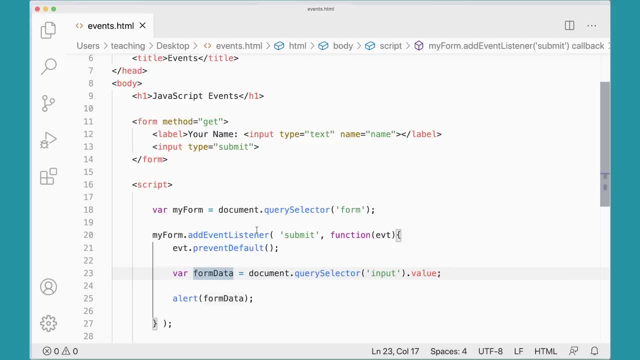 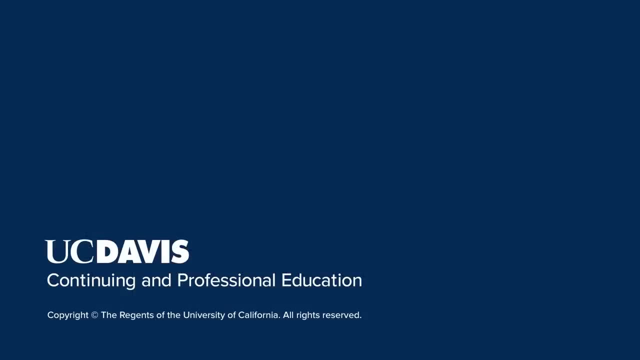 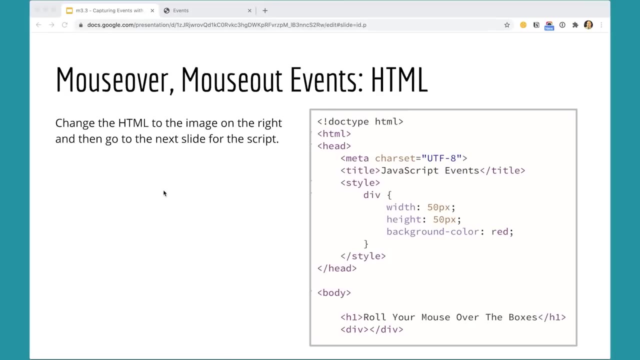 so that we can do what we want to do with JavaScript in here. It's very useful, Very, very useful. You know how to work with the click event and now you know how to work with the submit event. Now we can work with. 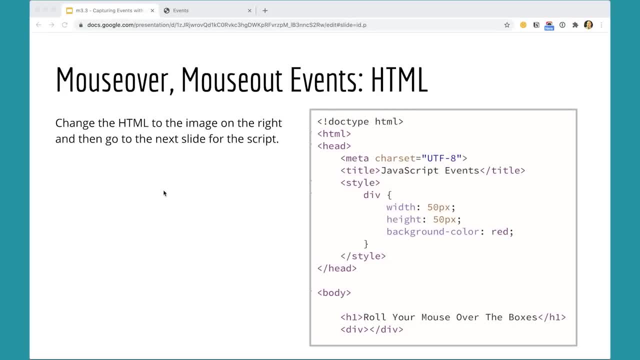 have some fun with mouseover and mouseout events in HTML and with JavaScript. So this is the HTML here. So create a page with this HTML in here And all I have is an H1 that says roll your mouse over the boxes and a div here. 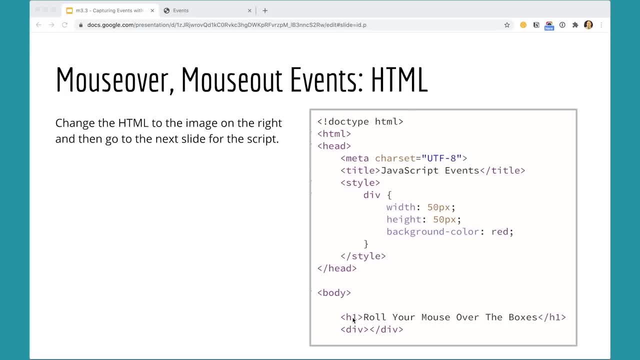 And we can roll our mouse over here, And we can roll our mouse over these two elements And what we're going to do here. I'll give you a second. You can pause this video and add this into the file. Make sure you add the style with the div. 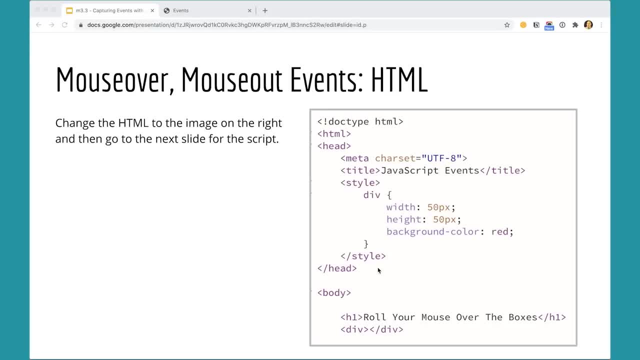 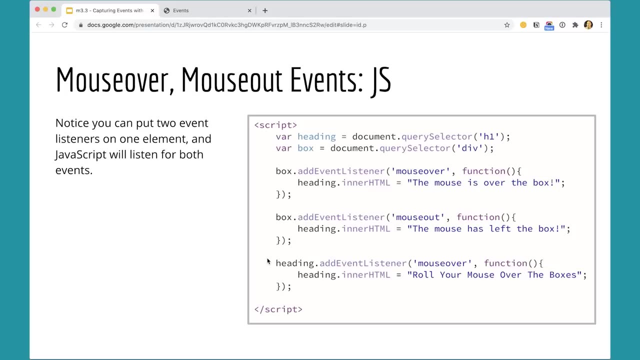 and set the width and height to 50 pixels and the background color to red, so we can apply this style and do some fun stuff with mouseover and mouseout. And now let's take a look at the script we can actually write to do this here. 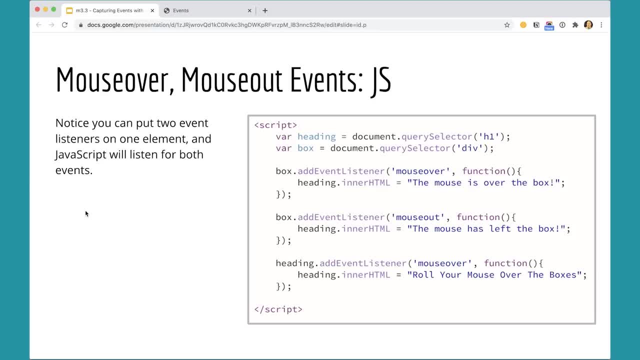 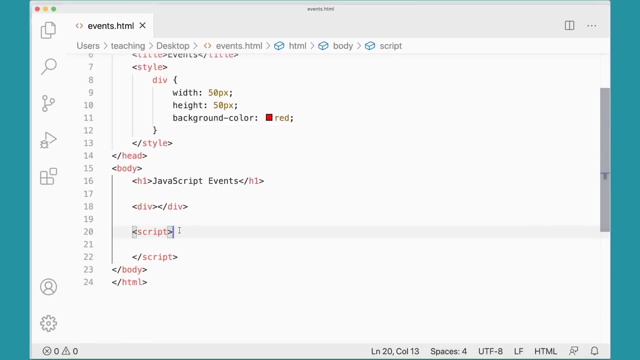 So let's go ahead and do this over here. So to begin with I'm going to make some variables for my heading and for the box to get those two elements. So let's start with that. So down here in my script: var heading equals document, dot query selector. 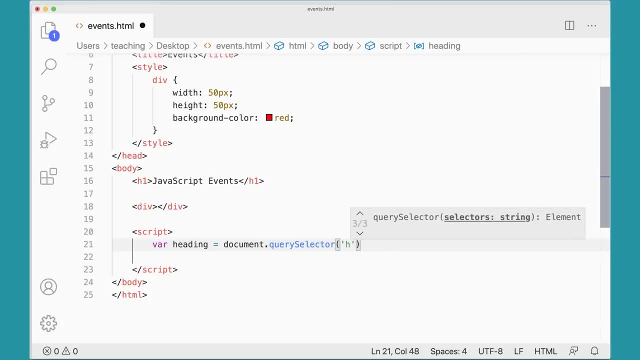 Each one And var. div over my. div equals document dot query selector div. So that will get those two elements there. I also want to change this text to roll your mouse over the box. Let's do that, And then let's just go see what this page is looking like. 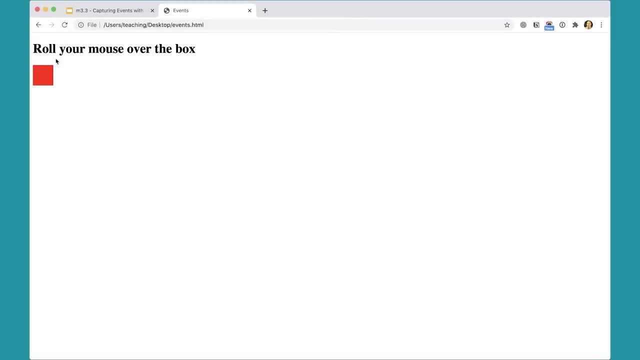 If I come over here and refresh this, I have a box and I have directions to roll my mouse over the box. So now I'm going to put an event listener on the box so that when I roll my mouse over the box it's going to change the inner HTML of this div right here. 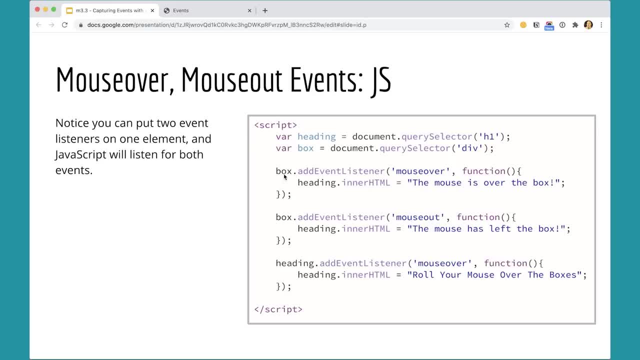 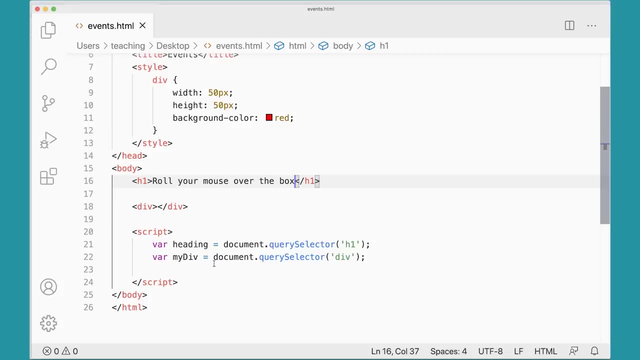 So we're going to add this here: Box out event listener. When we mouse over the box, we're going to change the inner HTML for the heading. The mouse is over the box, So let's do that. one Box dot add event listener. 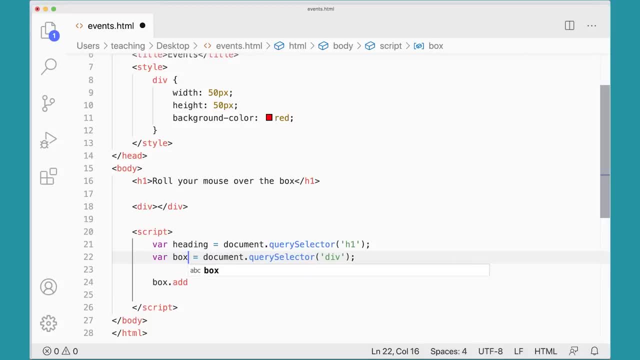 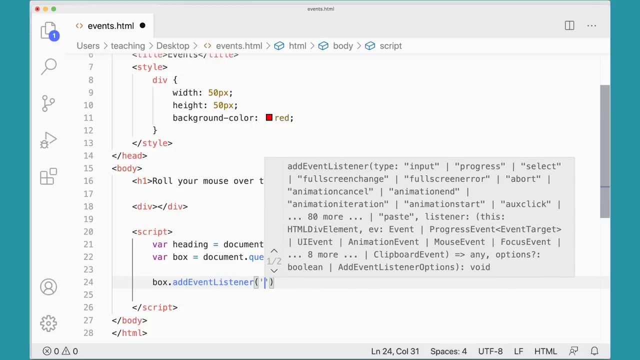 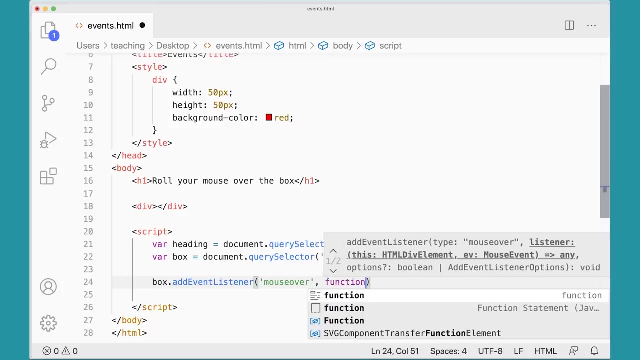 I guess I should have called this box to make this match my slot Add event listener And we're looking for a mouse over event And then, when that happens, we're going to run a function Like: so: We'll put the cursor in here. 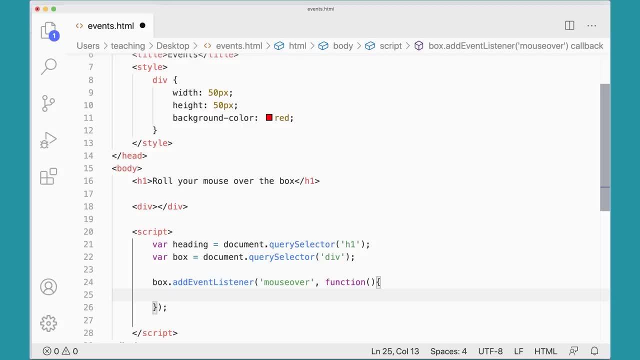 And then we're going to say, okay, when we roll over that box, we're going to go get the heading and change its inner HTML And remember that's a property. So we use the equal sign And we're going to change it to something like: 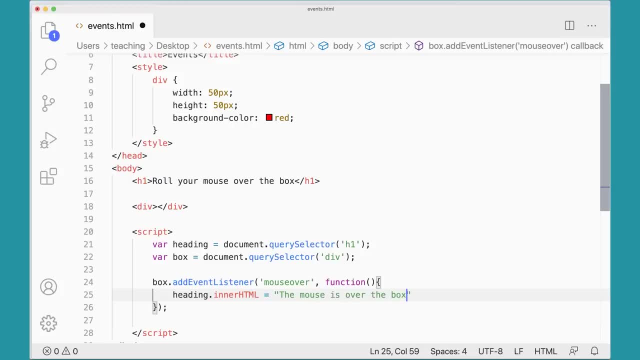 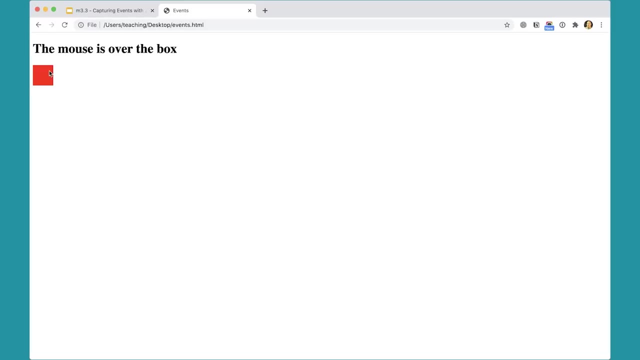 the mouse is over the box. Let's see if that works. Let's test that. And come back to my page over here Refresh. When I roll over the box, the mouse is over the box. Great, So that works. But now it's stuck there. 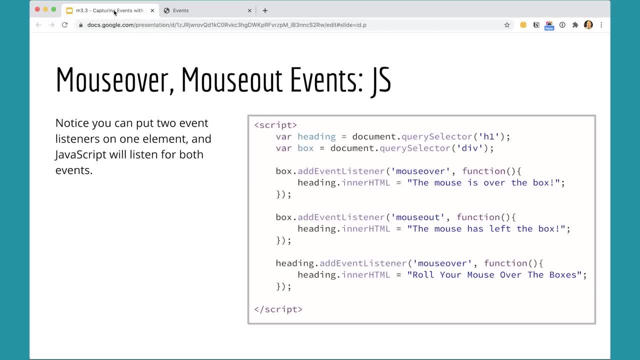 It's changed that content. So now I want to do something where, when I mouse out of the box, I'm going to put the. I'm going to change the heading to. the mouse has left the box, So it's another. I'm adding two event listeners to box. 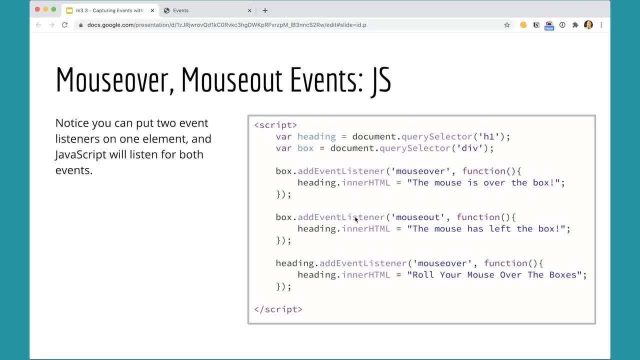 Both mouse over and mouse out, And this is part of the power of using the add event listener method is that we can have multiple. we can be listening for multiple events in one object, which is really kind of handy. So let's do that. 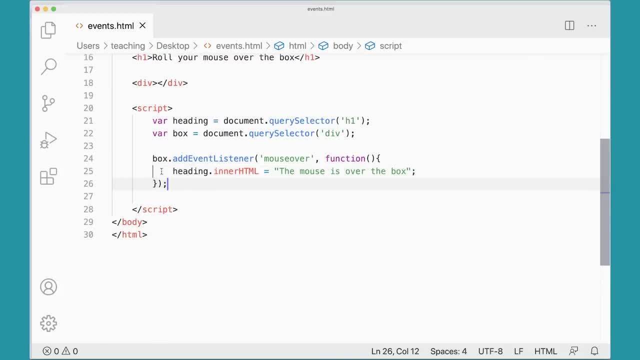 I'm going to come back here And, rather than take this off from scratch, I'm just going to copy paste, change this to: I'm going to take the mouse out. The mouse has left the box. Cool, That's great. 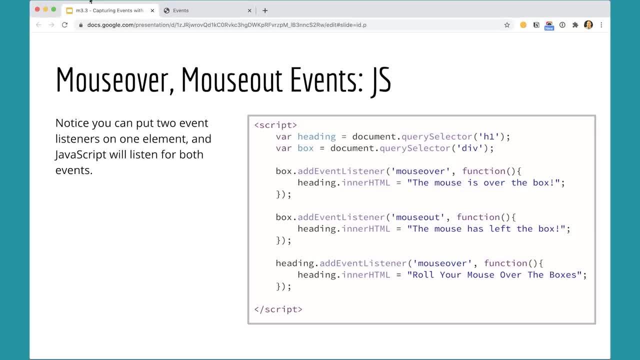 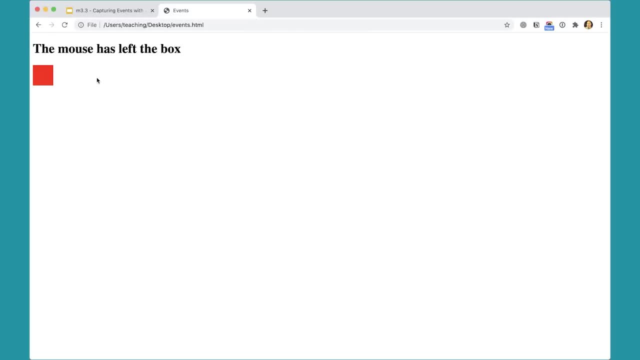 Let's go give that a try. Roll your mouse over the box So the mouse is over the box When I leave the box, the mouse has left the box. Mouse is over the box. Mouse has left the box, So I can go back and forth. 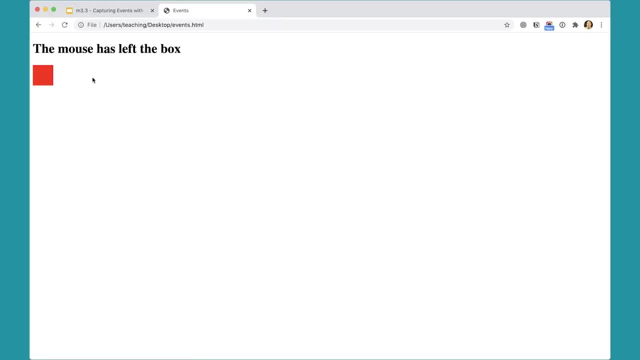 But it'd be kind of nice if I could return the page to its default state without having to click the refresh button, And so I'm going to add one more event listener for the header. So when I roll over the header it puts the original text back in there. 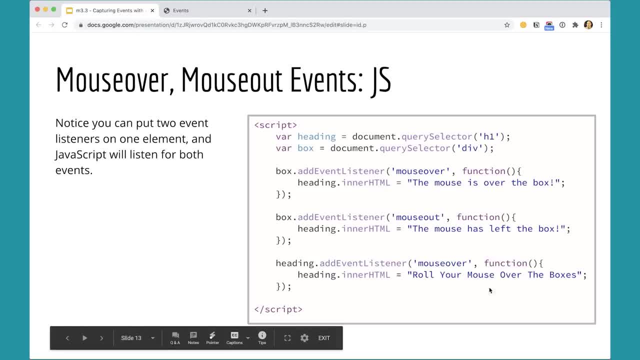 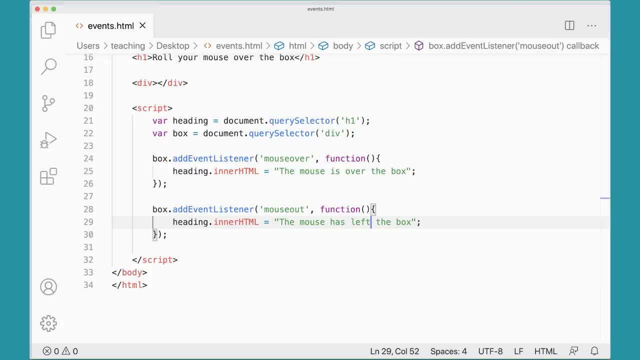 Like this: Roll your mouse over the box. I have boxes there, but really there's one box. So, yes, let's just fix that right here And I'm just going to copy this and paste it, But I'm no longer working with box. 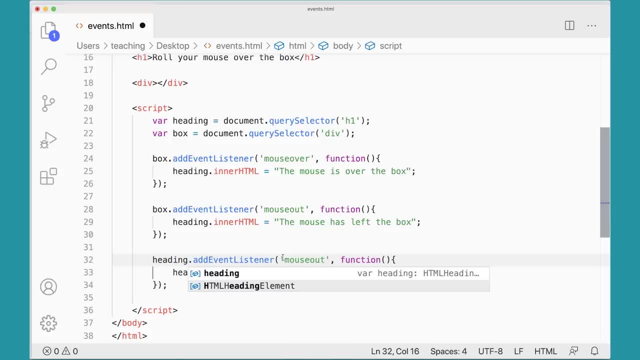 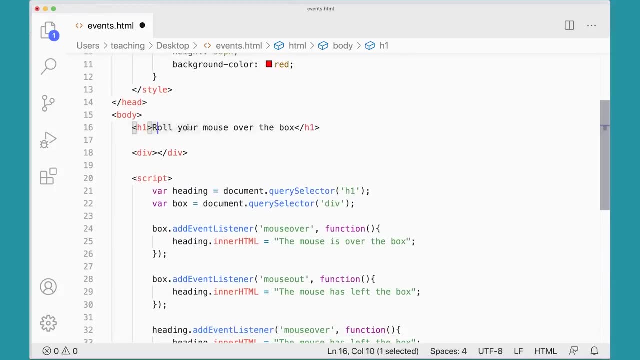 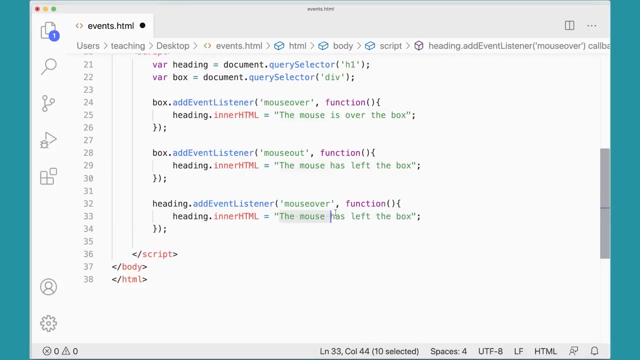 I'm going to put it on heading Add event listener: Mouse over And I'm going to put the same text that I have here in here for the heading to put it back to its default state Of where it was before. Let's give that one last try. 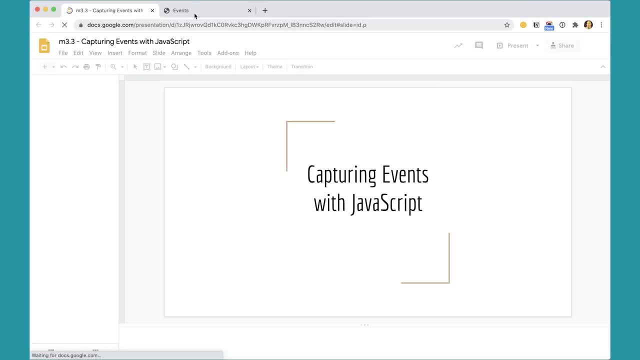 See if it's all working right. Oops, Refreshed the wrong page there, But now I can roll over the box. Roll off it And the event listeners are working. If I roll over the header, it puts it back to its original state. 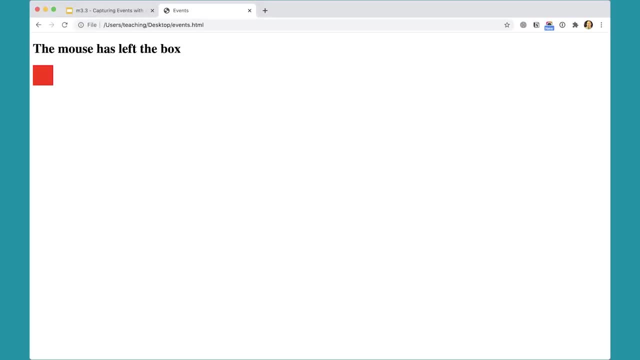 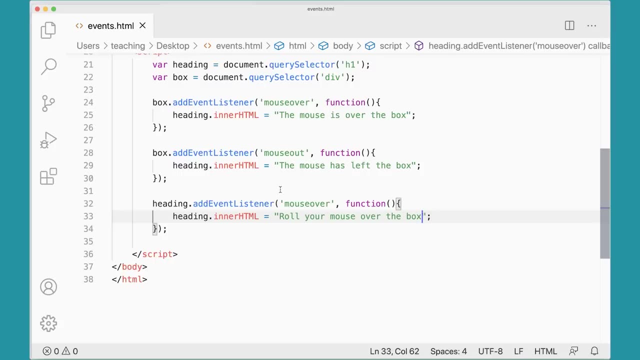 So this is a really great example of how we can use event listeners and mouse over and mouse out to change content on the page. Plus, you're making use of the inner HTML property, that element property, that's taking that element and actually replacing the HTML inside of it. 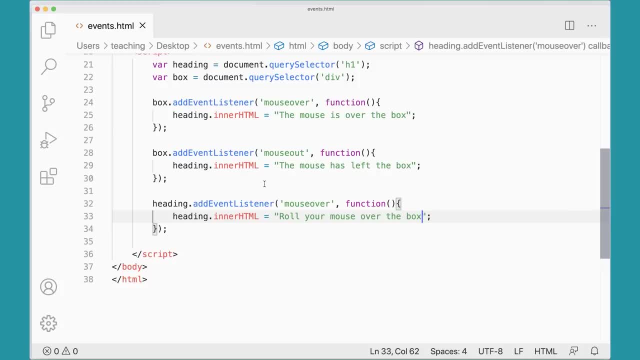 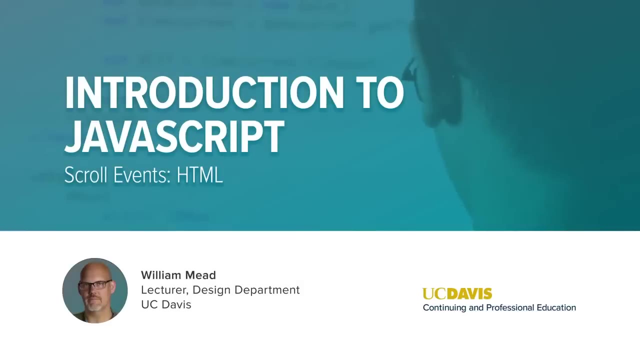 with something else which is really really very powerful and kind of fun. So now you're starting to see we can actually do some interesting things to web pages And we're no longer just putting stuff in the console. The next event type that we can look at capturing. 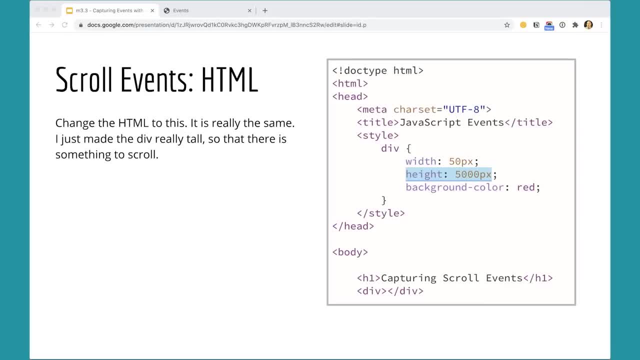 are scroll events, So change the HTML on the page that we just had to something like this: I've just changed the height to 5,000 pixels for this div. that's on the page, So I've got capturing scroll events and just an empty div. 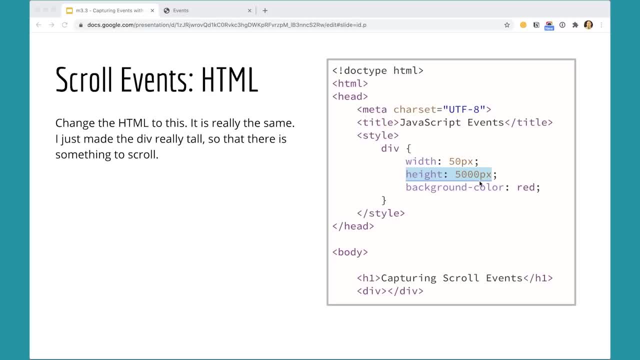 that's set to 5,000 pixels high. And I've set it to 5,000 pixels high so we have something to scroll. Otherwise, there's nothing to really scroll and we can't really capture that event. Okay, great. So once you've got that in place, 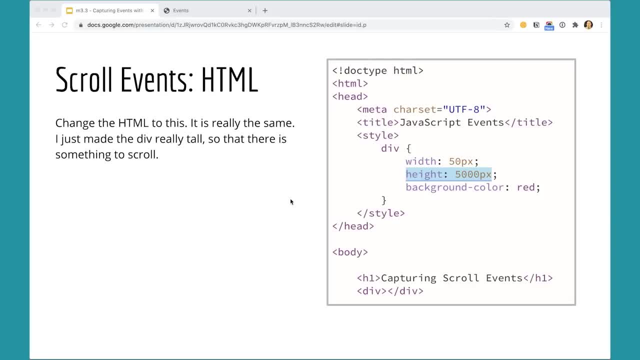 and you can pause this and go ahead and put that in there, so that you've got that HTML in place and that CSS in place. Once you've done that, we can go ahead and take a look at the script for capturing scroll events. And here we go. 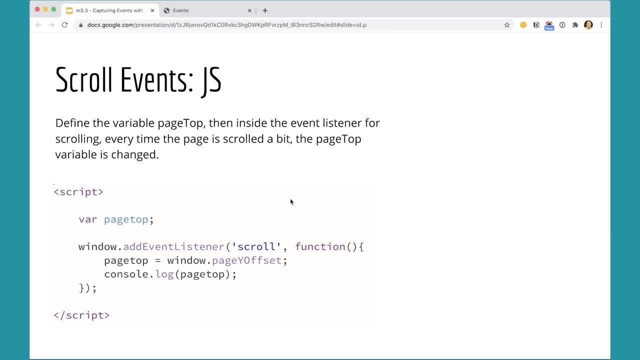 So I've got a script here and it's really pretty simple. It's a pretty simple script, but we're going to capture the scroll event and see what we can do with it, So let's try this out Over here on my script. 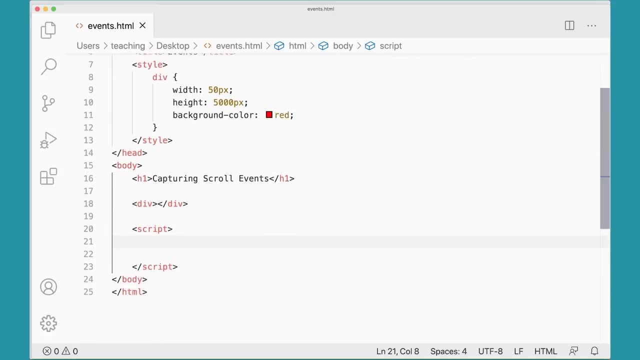 the first thing I'm going to do is create a variable called page top, And this variable is undefined at this moment. I've created a variable, page top, And then I'm going to create an event listener And the event listener in this case. 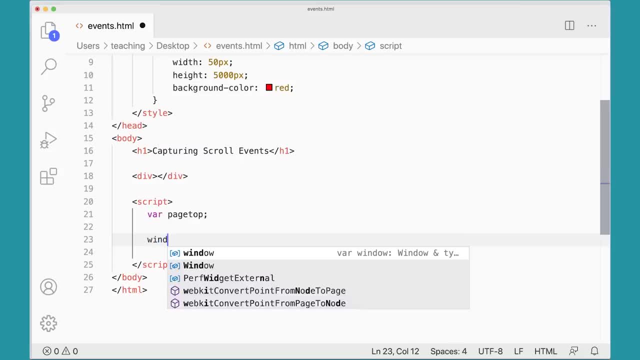 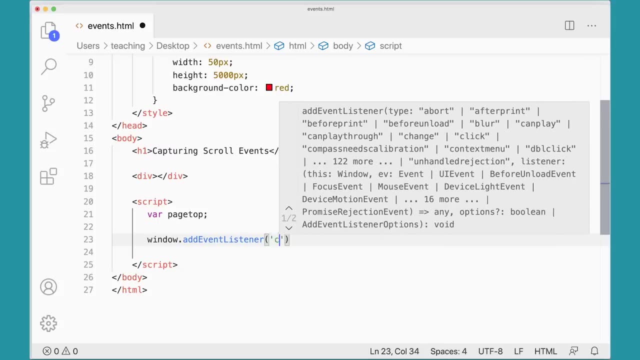 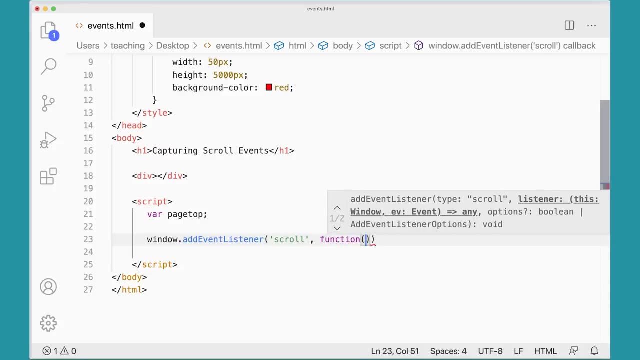 is going to go on the window object So I can actually do windowaddEventListener So I can listen for events for the window and I can listen for scroll scroll event. And then I'm going to run a function When the scroll event happens. 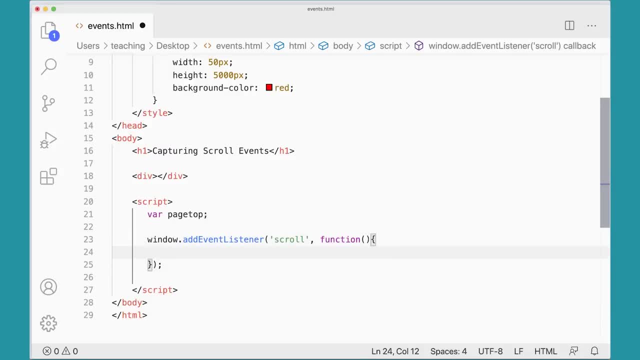 Okay, So we've got a function that's going to run here, And what I want to do here is I want to take page top and update its value. It started out as no value at all, But I'm going to update the value of page top. 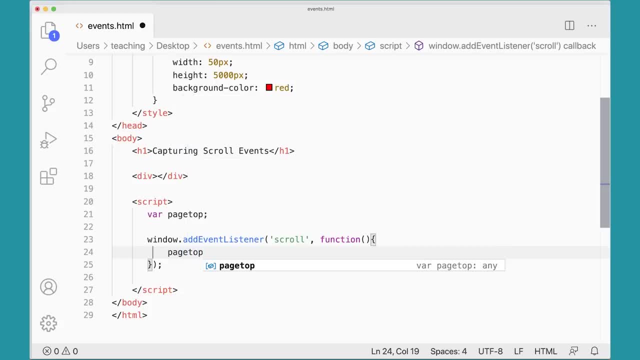 Page top is going to be equal to window page y offset, So we're going to set it to that And then I'm just going to console log out page top For now, Just so we can kind of see what's going on as we're scrolling the page. 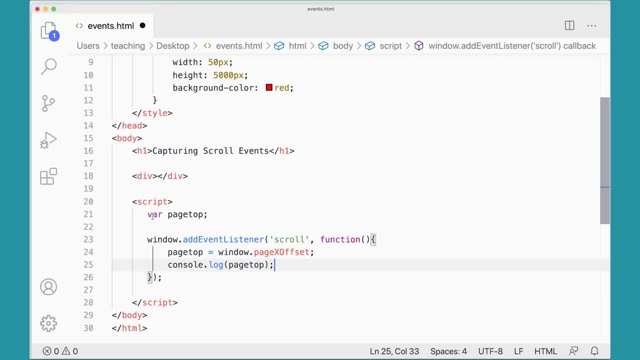 So a couple of things you might be wondering. One is: why am I defining the variable here? I could just put var there, But let's stick with this for the moment And then I'll come back and answer that question once we see what this does. 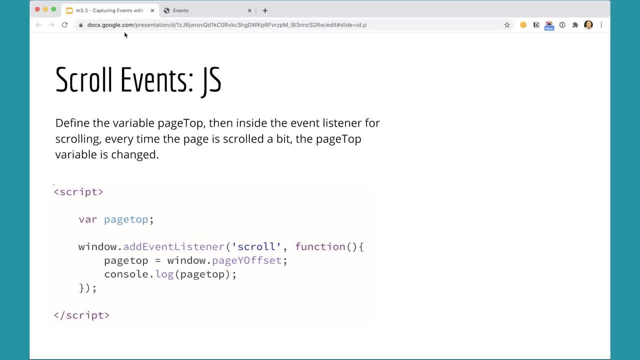 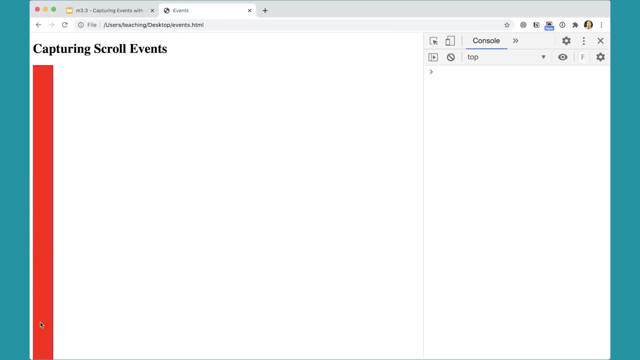 I'm going to go over to my browser over here And here's my page. I'm going to refresh that And here's my div that's 5,000 pixels tall. I have my inspector open and the console selected over here. 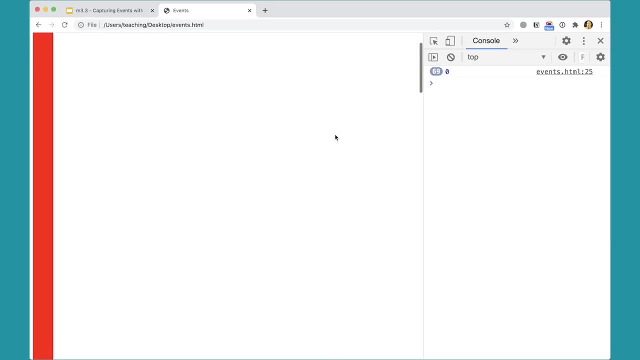 So I can actually see As I scroll my page. It's capturing that thing here, But it's not working right. I can see that the script is firing, But my zero is not changing here. What did I do as a mistake? 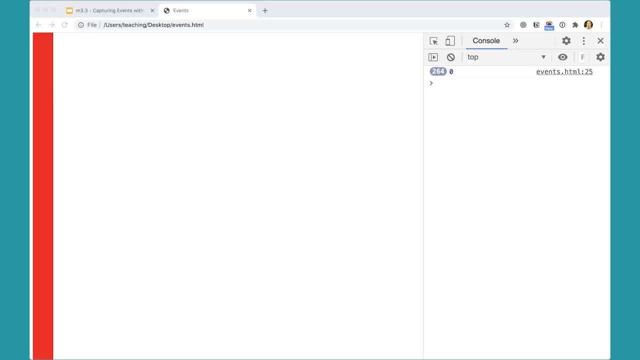 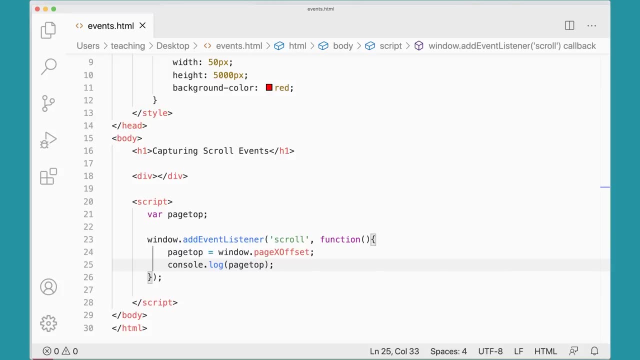 Let's go take a look at my code. This is a really great example of something I did wrong here, And this happens all the time. This will happen all the time. This will happen to you, Don't feel bad. I'm kind of glad this kind of thing happens here. 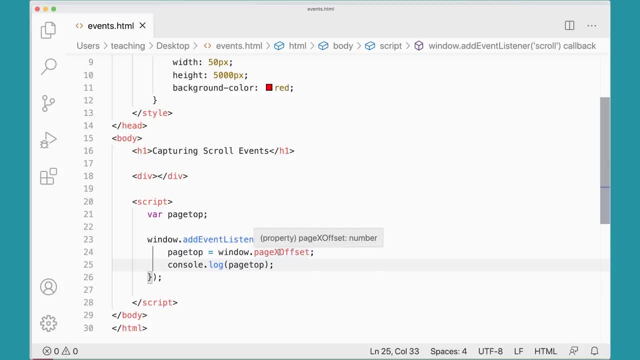 Notice. I set page X offset. That's going to keep track of whether the page is moving horizontally or moving left and right horizontally. Page Y offset is the one that I wanted And you may have caught that, as I was saying it earlier, that I typed in the wrong thing there. 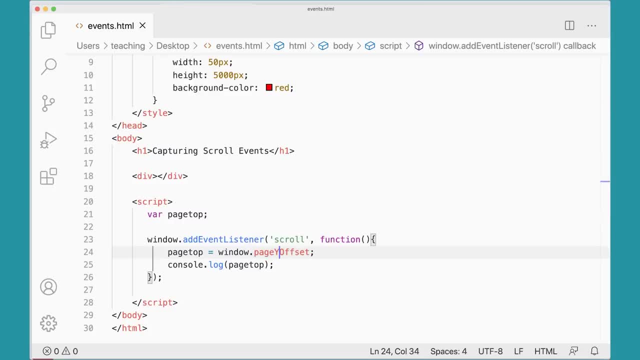 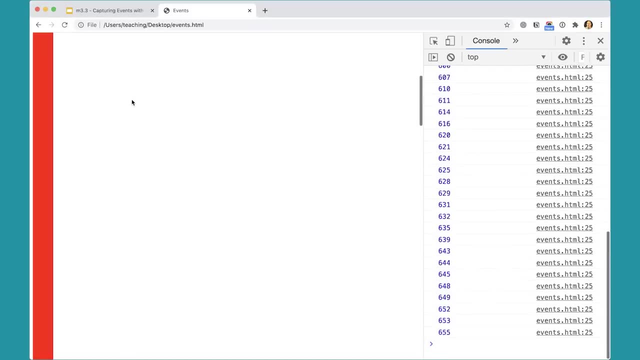 But I'm going to change that to page Y: offset here And now. let's go see if that works properly. Come back here, refresh my page And you'll notice as I scroll it's telling me how many pixels down I've scrolled. 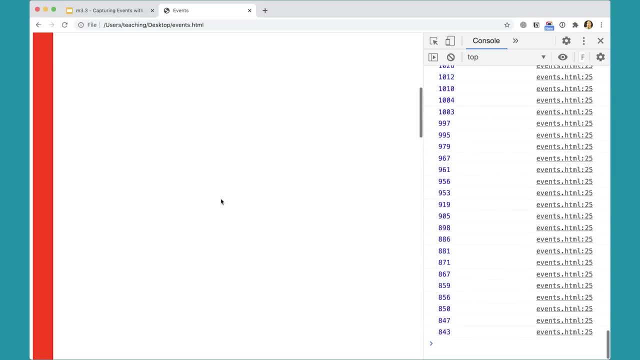 I can scroll down or I can scroll up And you'll notice as I scroll up the numbers will get smaller because the page Y offset is telling me how far from the top of the page am I down the page here And I should be able to go down to 5,000. 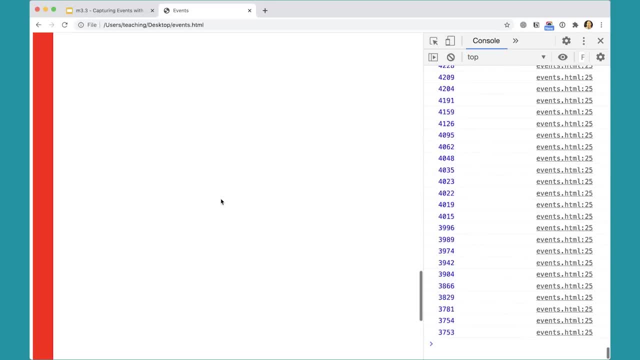 because I made my element 5,000 pixels. Not quite 5,000 at all there, but you get the idea. Now, one thing to note here is that this, this event listener is firing very, very often. Couple things to note. 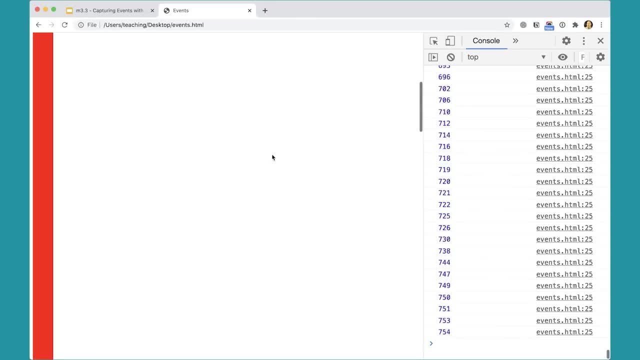 It's firing. very, very often It's firing every time I scroll just a little bit, This event listener is going one, two, three, boom. Every single time I scroll just a little bit it's firing that event listener. So that makes the scroll event listener. 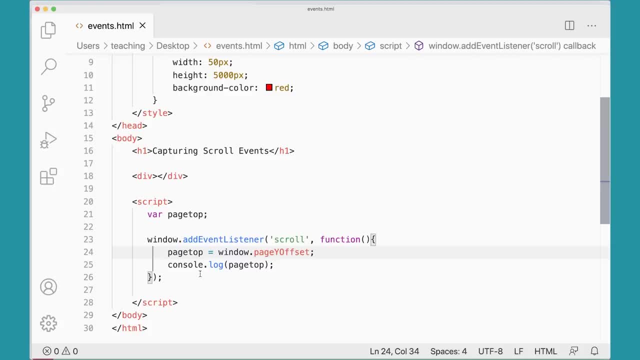 very expensive in terms of processing and you know the kinds of things that JavaScript is doing. So you need to be very careful with the window at event listener scroll event- because it's going to fire frequently. That brings me back to this. I could have just put bar page top here. 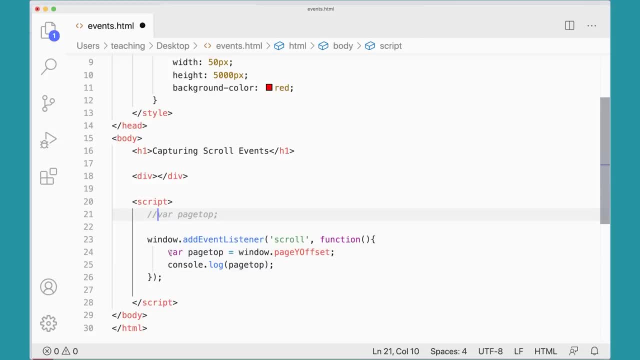 Instead of defining it here. But every time I scroll just a tiny little bit, it's going to recreate. It's going to ask JavaScript to recreate the page top variable from scratch and then assign a value to it, Whereas if I do it up here, 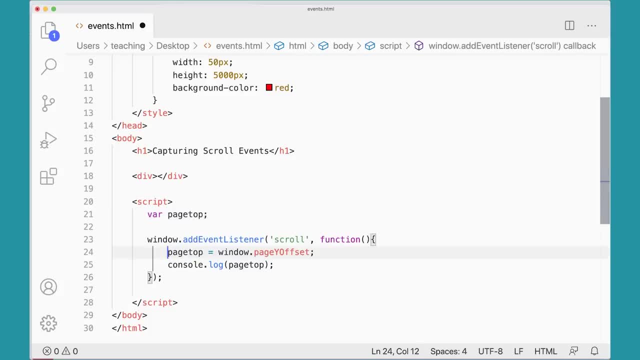 it's a little bit less expensive because now I'm just updating the value of page top. I create the variable once and then update the variable as I scroll down the page. It's not a big difference. You're not going to notice a huge difference in this example. 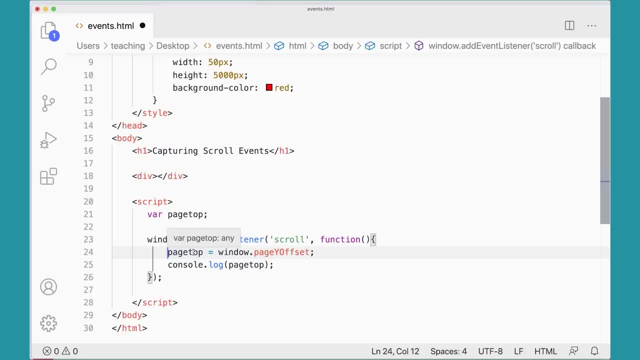 But it's kind of important to mention because when we talk about creating events that are about scrolling the page, we need to be really careful about what we're asking JavaScript to do, because your page can get bogged down really quickly, keeping track of all of these scroll events. 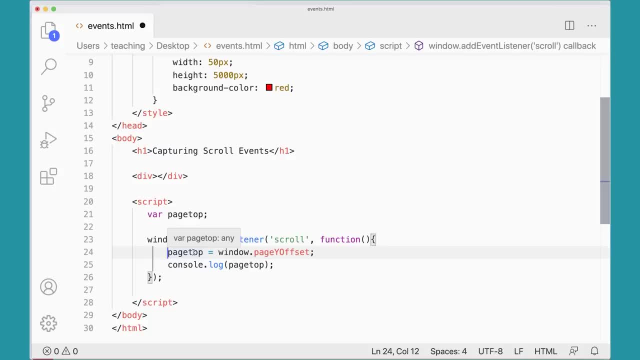 that are happening And there are some techniques you can use to sort of mitigate the effects of that, And we'll look at some of those later in this course. Okay, but for right now, all I want you to be really aware of is that we can actually capture. 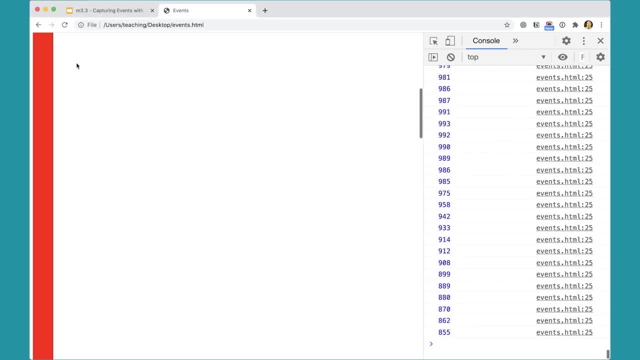 the scrolling of the window in this way. that's very effective here. Let's scroll back up to the top and refresh and scroll down and see it's capturing these numbers. So this is actually a really effective way of doing it. One last thing I want to mention. 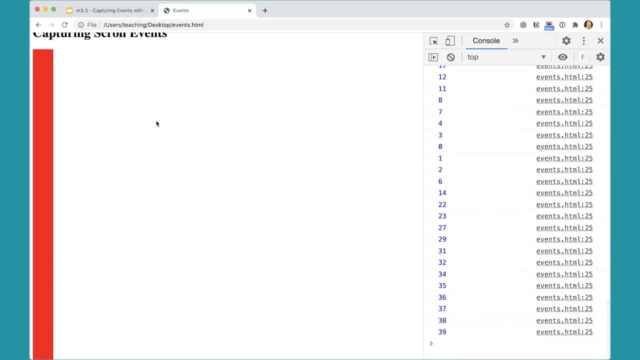 while we're here about the scroll event is notice it doesn't capture every single pixel. If I scroll slowly enough I'll capture a lot of them, but you can see I've missed a few of them in there If I scroll really fast. 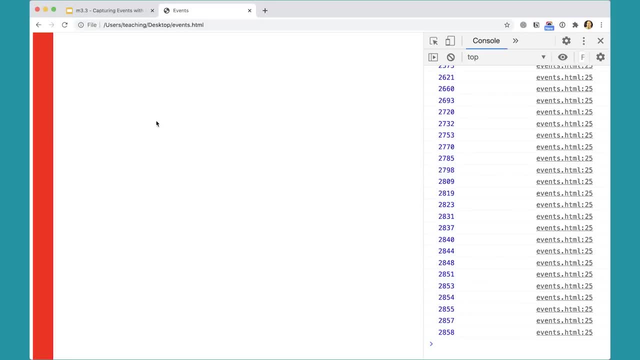 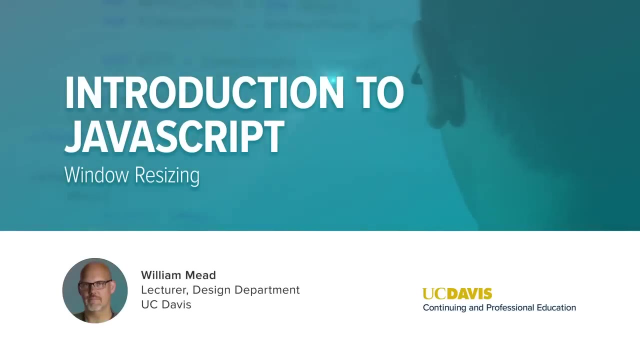 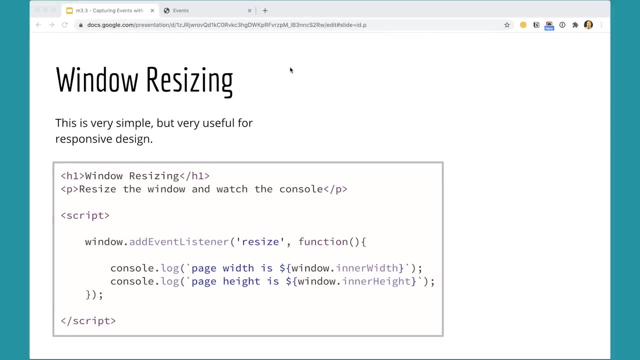 it'll skip lots of them more frequently. So that's another thing to pay attention to. If you're looking for a very specific pixel, it's harder to get with the scroll event. Another simple example that we can look at is watching for a resize of the window. 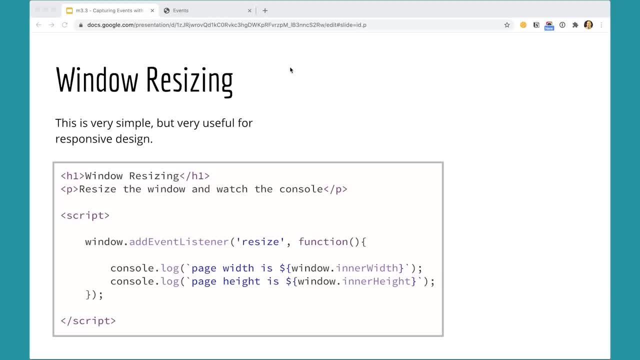 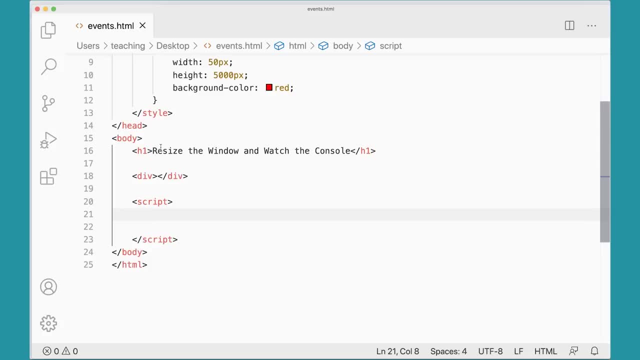 And this is useful in responsive design. So let's take a look at this one really quickly as well. I have an H1 year. resize the window. I don't need my div anymore. I can get rid of that, And I can also get rid of my style tag up here. 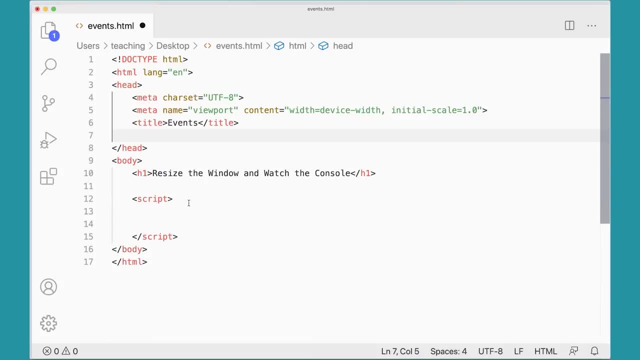 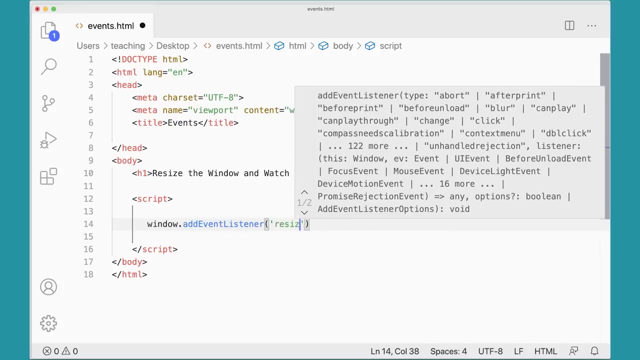 the whole style tag. We don't really need that anymore either. But down here I can actually do another windowaddEventListener, But in this case the event we're going to look for is a resize. I'm looking for a resize of the window. 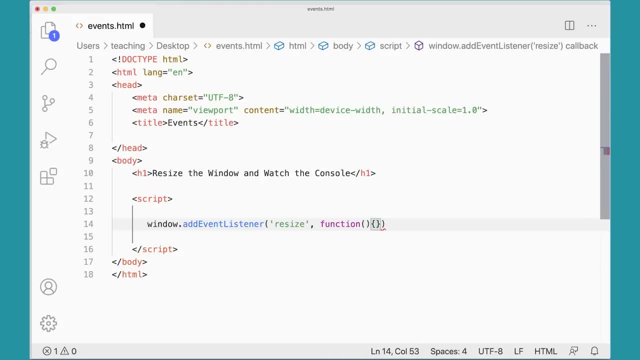 And we'll run a function And then I'm just going to add two consolelog statements in here so I can watch for resizing both the width and the height of the window. So I'm going to do consolelog parentheses And in here I'm going to use my tick marks. 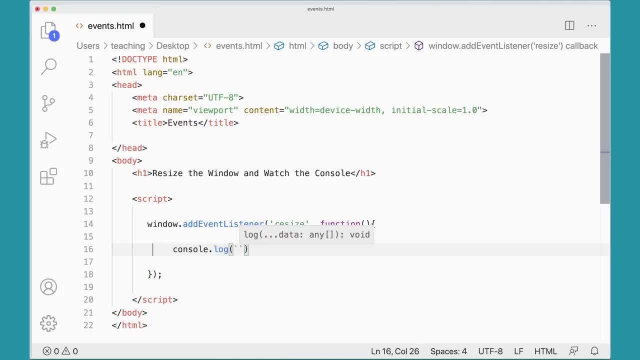 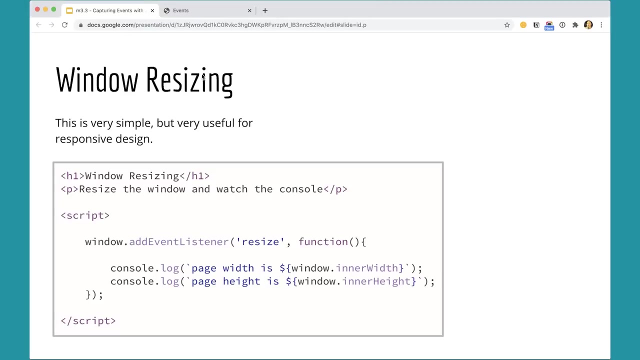 and put in here the window width is- I think it's windowinnerWidth, Is that right? Let me check my slide over here: windowinnerWidth, yes, And windowinnerHeight, windowinnerWidth, And that's a variable. so I'm going to put a dollar sign. 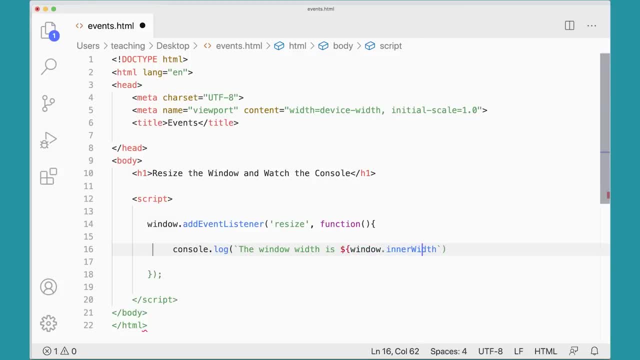 and a curly brace, And at the end I put curly brace, And then I'm going to just copy this consolelog here. So I'm going to type it all again and paste it in here: windowwindowHeight- windowwindowHeight. 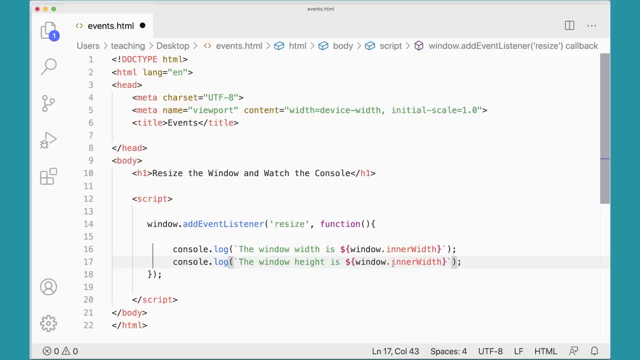 windowwindowHeight, There's windowinnerHeight. InnerWidth and innerHeight are properties that belong to the window, So we can actually get a number of pixels for the window with this, And that will actually work pretty nicely. So those are a couple more properties. 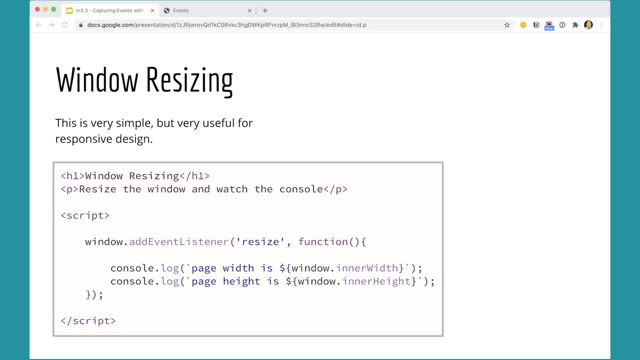 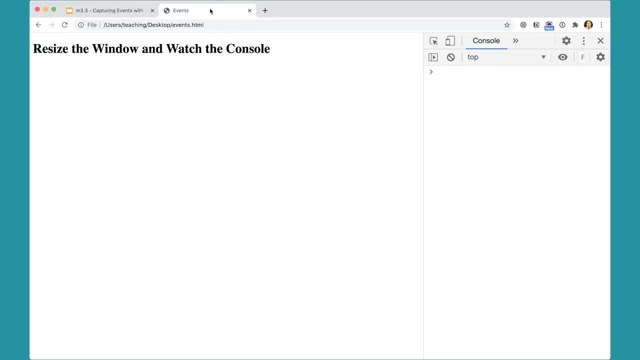 to add to your list of things, list of properties that you know about. So I can come over here and go to my events page. So I can come over here and go to my events page. I'm going to refresh this And if I actually pull this off of here, 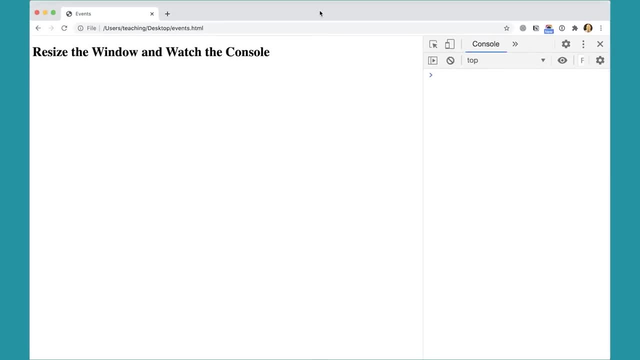 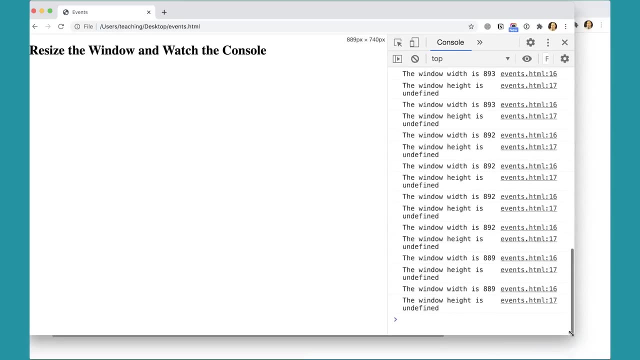 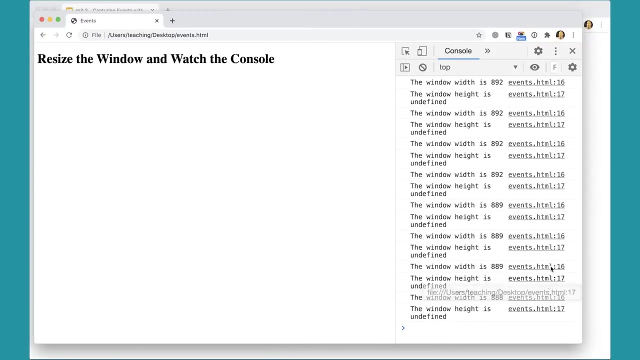 and let me see if I can position it just right here. There we go, And then I'm going to resize this window, And as I do that, you can see that I'm getting some comments over here about how wide and how width. 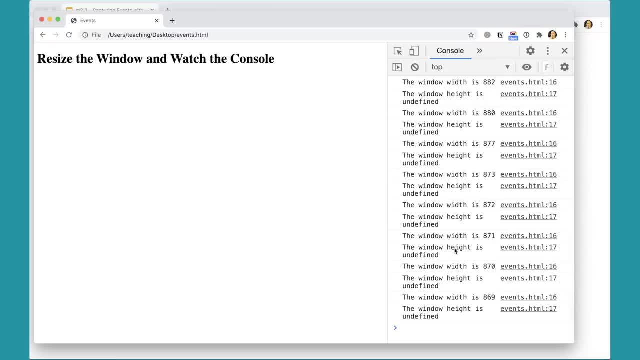 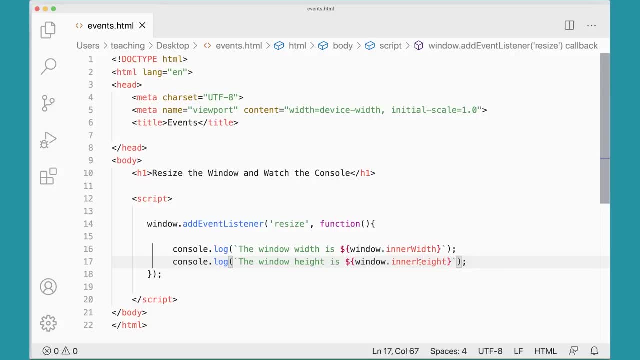 windowheight is undefined. windowheight is undefined. Well, I did something wrong with my windowinnerHeight. Well, I did something wrong with my windowinnerHeight. Let's go see what I did wrong over there: windowinnerHeight, windowinnerHeight, capital H. 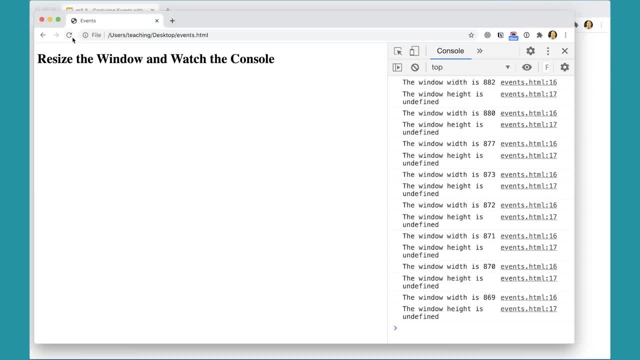 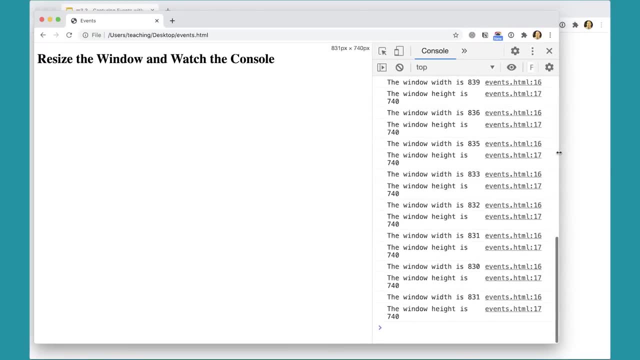 And there we go. That happens, Happens to the best of us, And now let's try it again. All right, So now I'm getting, the width is changing because I'm changing the width here, And then, if I come down here, 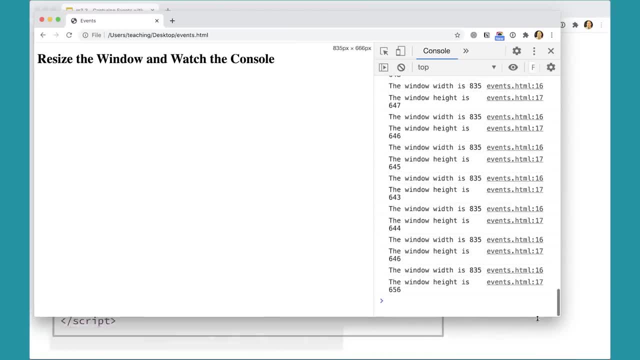 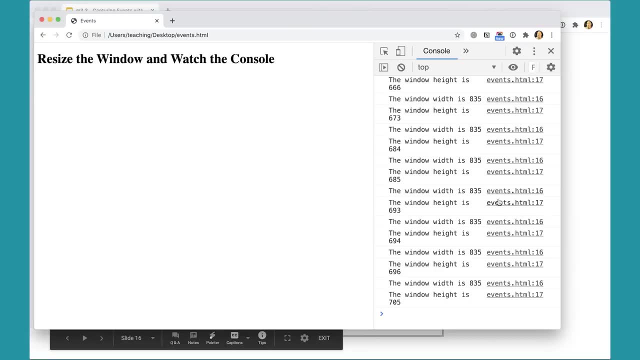 and change the height, you can see the height is changing. So there we go. We have a tool that we can use to find out how wide our window is and how tall our window is, And this is extremely useful in JavaScript, And the resize event can be very useful too. 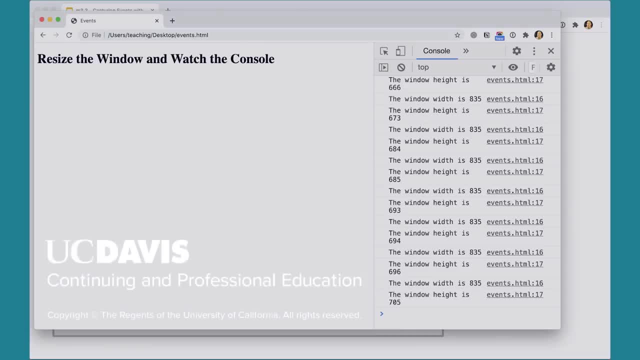 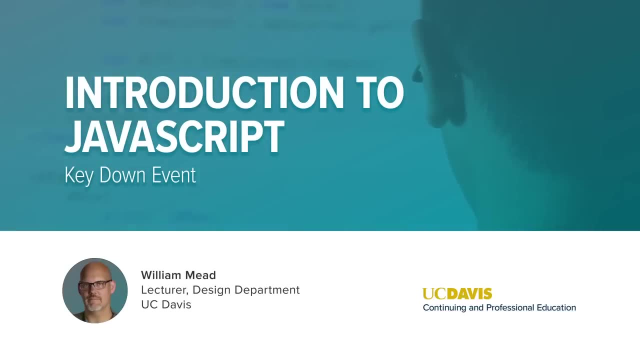 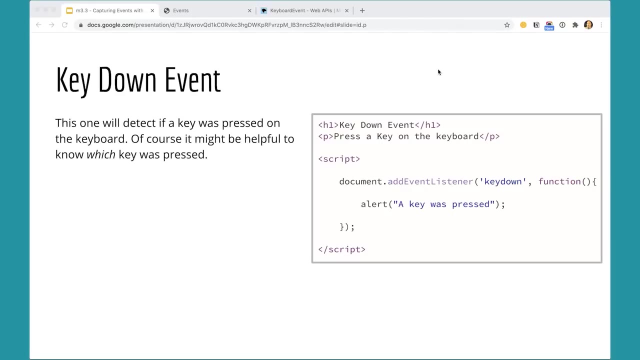 if you're doing something with responsive design. The next type of event that we're going to capture is when you've pressed a key on your keyboard, So that's kind of interesting that we can capture that. Imagine creating games that you could play where you're pressing keys on your keyboard. 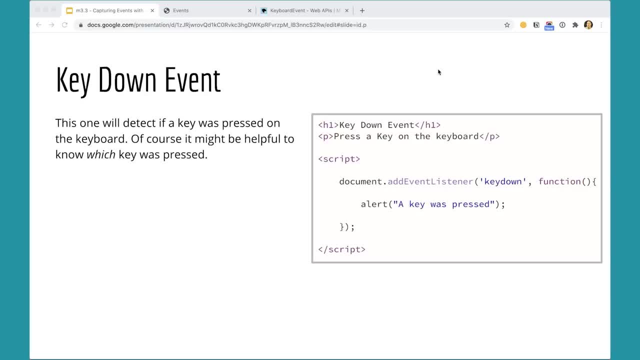 and things happen in the browser or something like that. That would be kind of fun. So over here on your HTML page we can just add a script, But this time we're going to actually attach the event listener to the document itself. 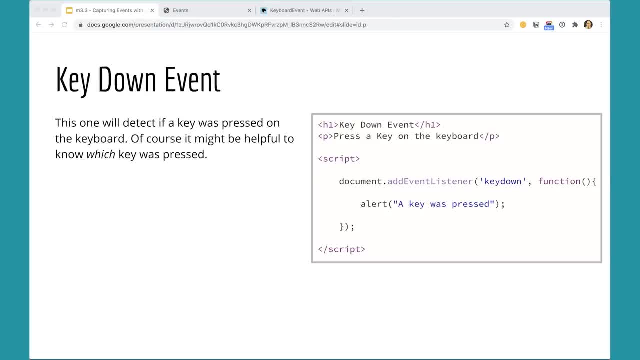 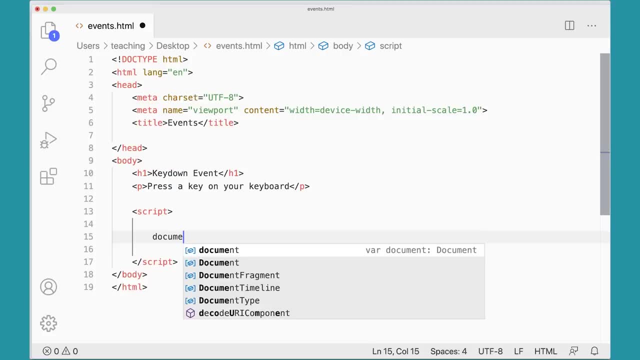 So let's just do that. It's kind of a really simple thing to do. So let's come over here And I've got key down event, press a key and I'm going to actually say documentaddEventListener And in here I'm going to look for a key down event. 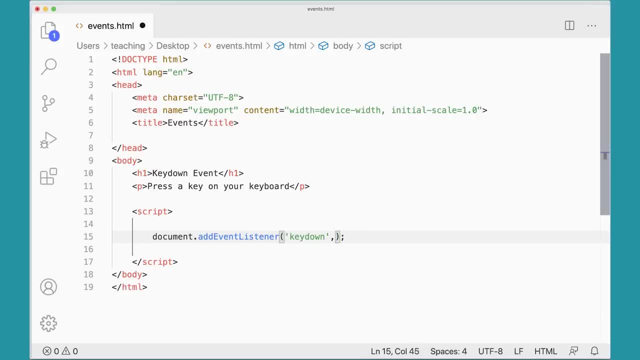 You could also look for key up or some other types of events. They have to do with keys as well, Function, And then I'm just going to alert: A key was pressed, Okay, great. So let's go over and give that a try. 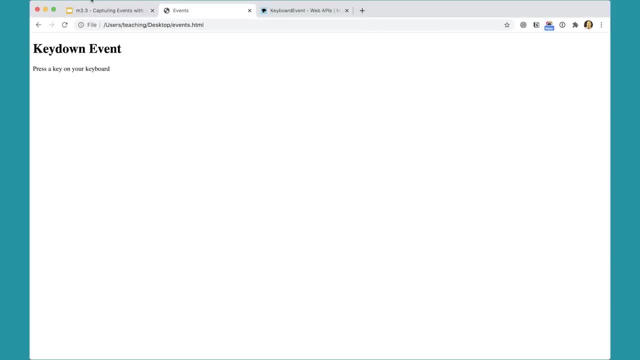 Over here. if I refresh this page and press a key, I get a key was pressed. That's cool, So that's working. great. I can detect when a key was pressed. Now we can check to see that a key was pressed. 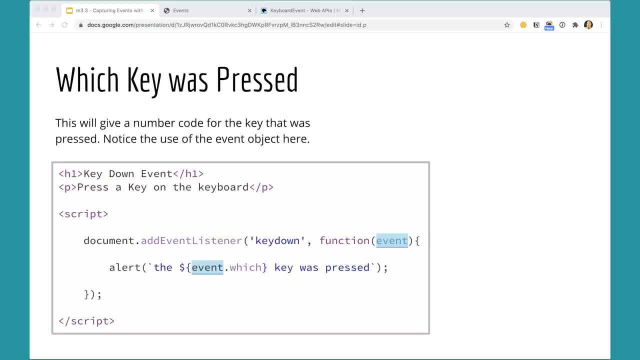 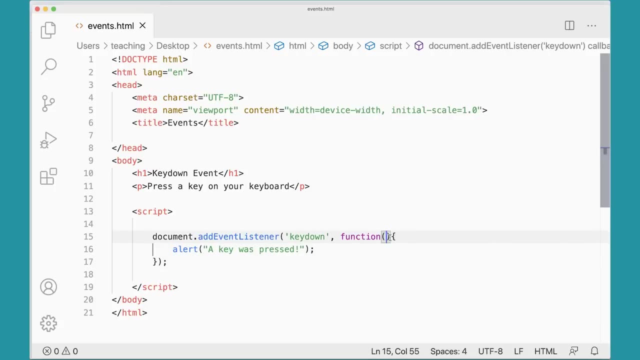 but it'd be kind of nice to know which key was pressed, And we can find that out through using the which property on our event. So let's give that a try real quick. So I'm going to pass in here my event object. 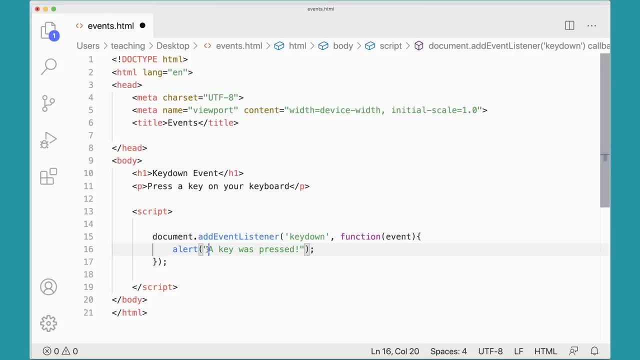 And then in here, instead of using my quotes, I'm going to use the tick marks And say the event dot, which key was pressed, And event dot, which is a variable. So I'm going to put a dollar sign and a curly brace. 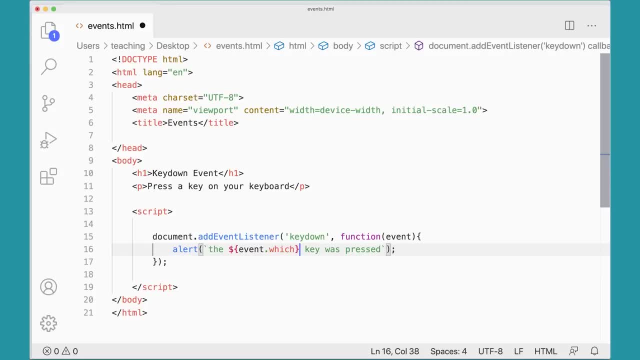 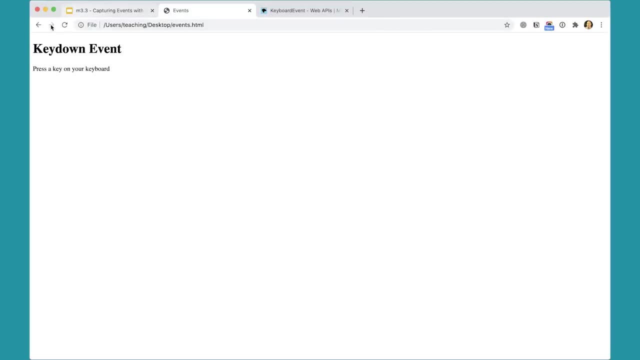 And then a curly brace, And let's give that a try. So now when I press the J key, I get the 74 key was pressed, So I'm getting a code that goes with each key. If I press the L key, 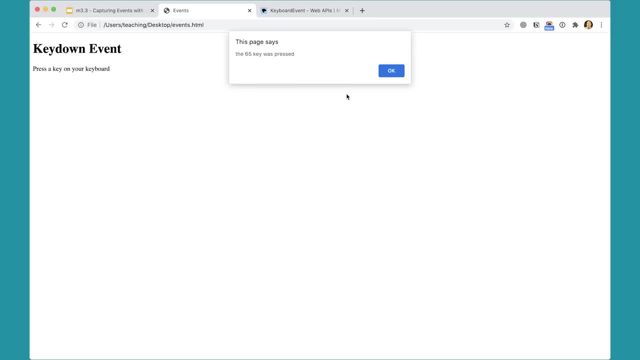 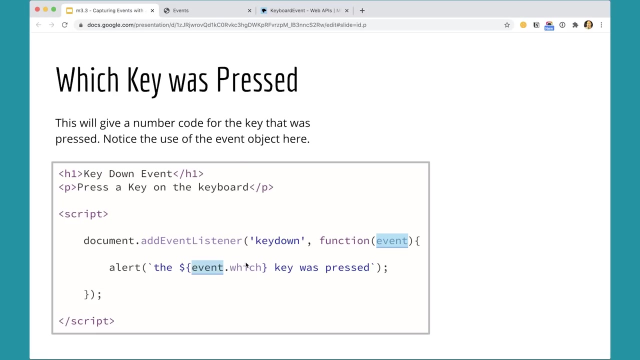 I get a 76.. If I press an A key, I get a 65. So I can do this kind of thing to find this sort of stuff out. Now, what's interesting here is that the which property has been deprecated- I just found out about this recently. 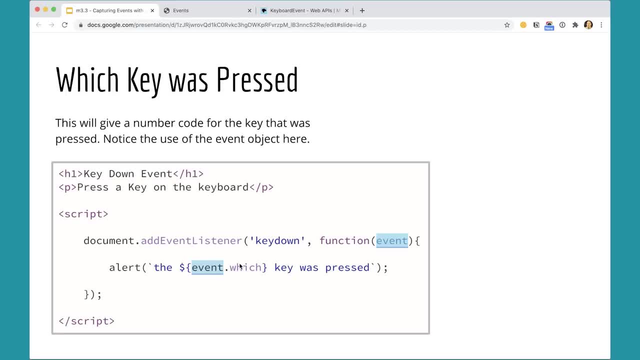 And so more recently than I put together this lesson. So this is something that happens with JavaScript and with web stuff in particular is that things change, And part of learning about the web is getting comfortable with figuring out, finding out when things change and what to do about it. 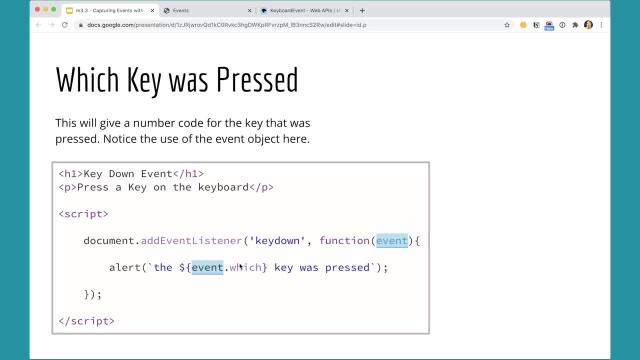 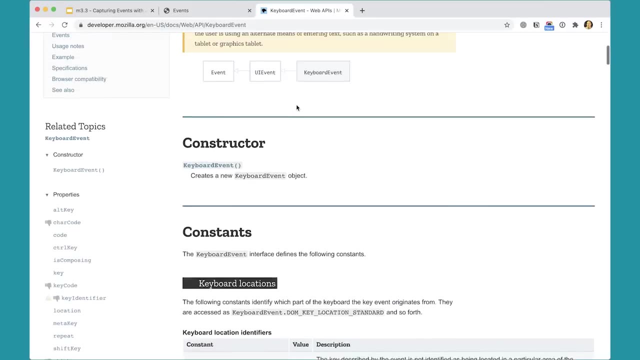 And, from my understanding, the which property was deprecated because keyboard layouts can change a lot all over the world, So they decided that that was not the good way to go, And if you come over here to this MDN page, you can actually find out a lot about. 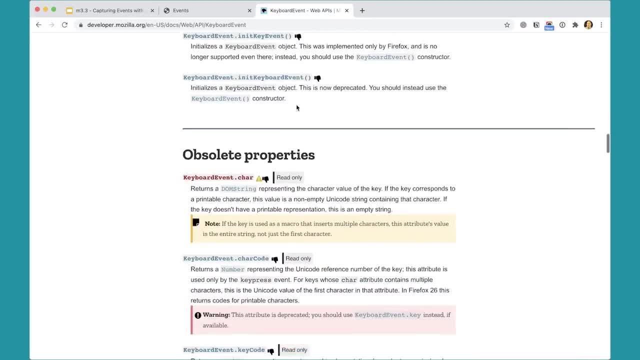 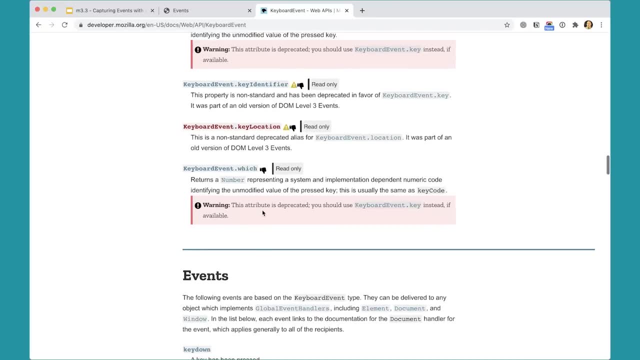 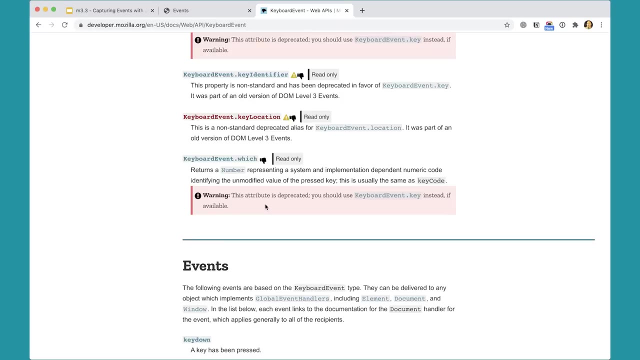 the different events And down here it'll actually say which the keyboard, which key has been deprecated. Now the reality is is that browsers will support it for a long, long time to come. You could certainly use it, but they're saying: 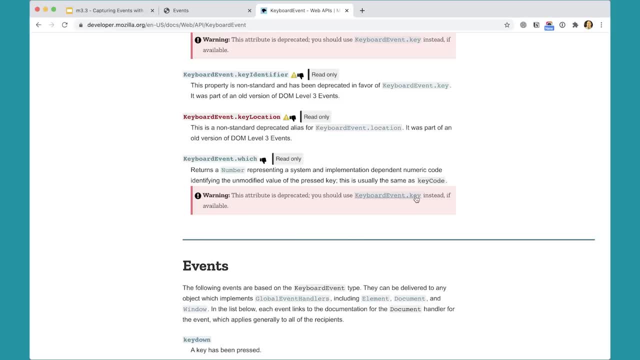 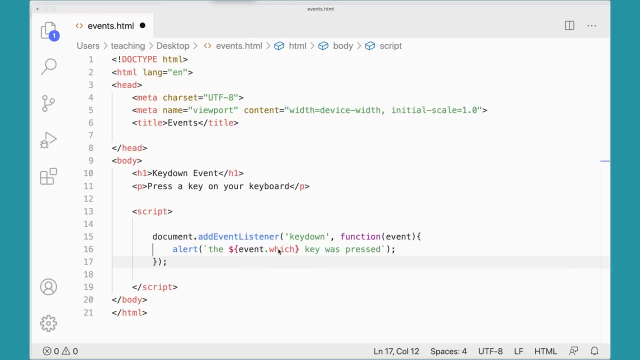 you know you shouldn't use that. You should use event keyboard key instead. So let's give that a try real quick. I'm back here on my page and I'm going to change which to key, Because that's what the MDN says I should do. 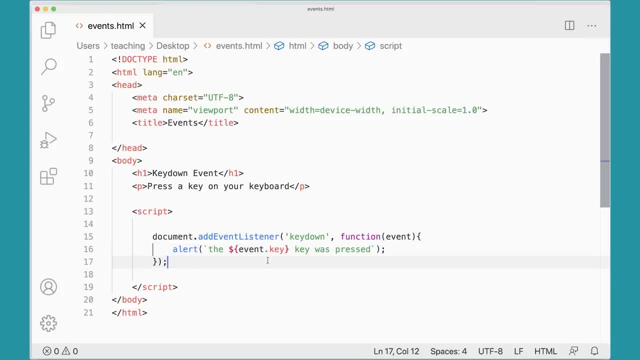 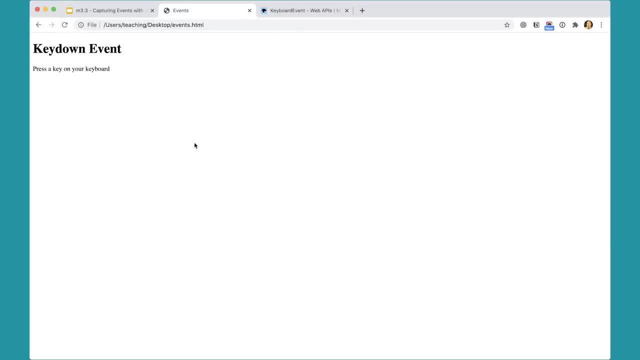 And they're sort of the most authoritative resource on this stuff. So let's go over and sort of check that out over here. I refresh my page. If I press the F key now, I'm not only getting not a number, but I'm actually getting the F key was pressed. 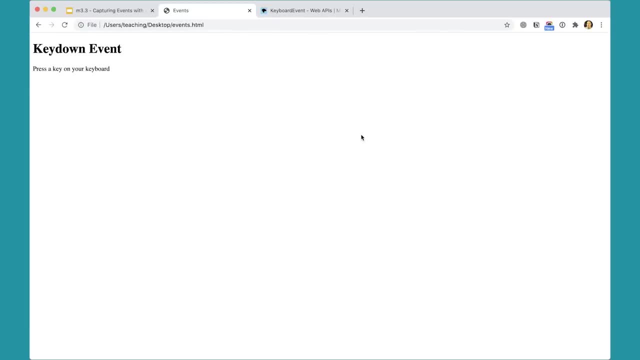 If I press a Y, I get the Y key was pressed, So that's kind of interesting and useful. We've captured a lot of different types of events now, from the click event to the submission of a form, to the mouse over and mouse out. 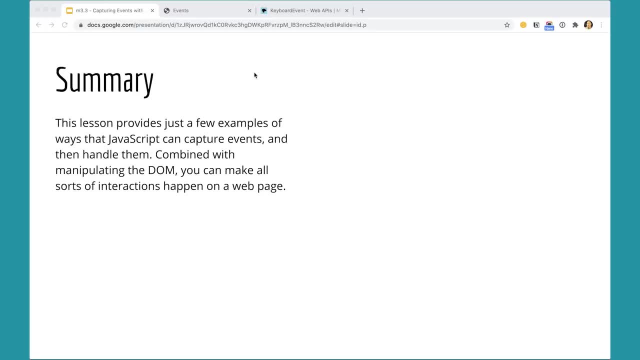 and scrolling and capturing keys. There are all types of events And these are just a few examples. There are plenty more events that you can capture. You can look up the full list on the Mozilla Developer Network if you want to sort of really poke through them all. 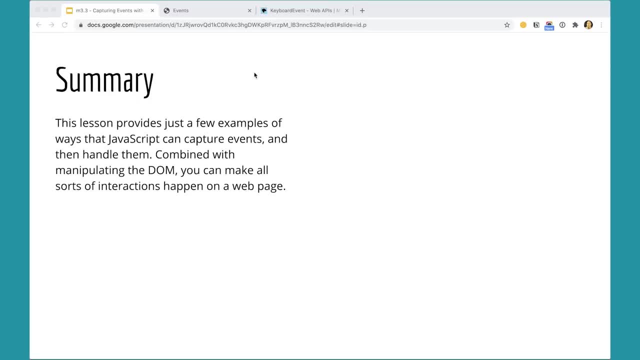 So, but these will keep you busy for quite a while- just these few events, And by capturing these events and combining that with manipulating the page, we can do some really interesting things in our web pages now, And you really have a lot of the basics that you need. 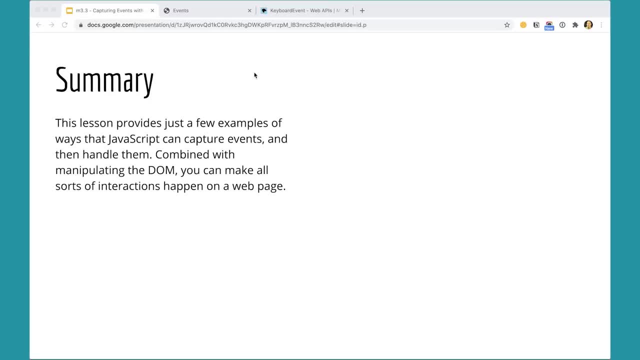 as a foundation to start building interesting interactive web pages. So we'll be going on from here and we'll be talking about a few more basic concepts and techniques, And then we'll be practicing a lot of this stuff and building some projects so you can actually try it out. 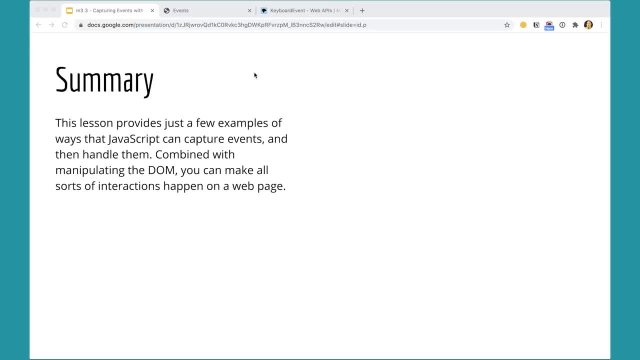 Plus, there's lots of challenges along the way- challenge exercises and challenges within the projects for building stuff- And hopefully you find it fun and are willing to come along with me on this journey and continue to put what you've learned with JavaScript to use and actually making some interesting, fun things. 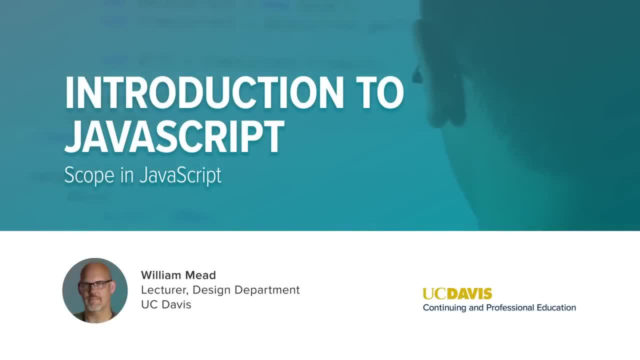 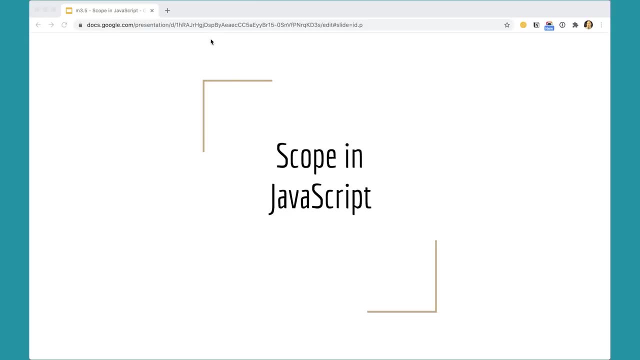 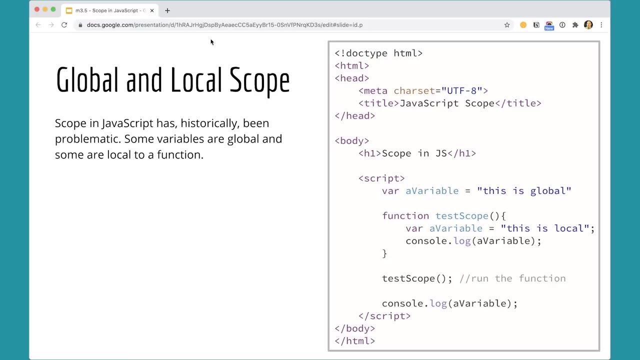 The next topic we need to get into is the way scope works in JavaScript, And this is an important thing to understand, Because in JavaScript, when JavaScript was originally written, you have to keep in mind that they really thought that it was going to be very short scripts. 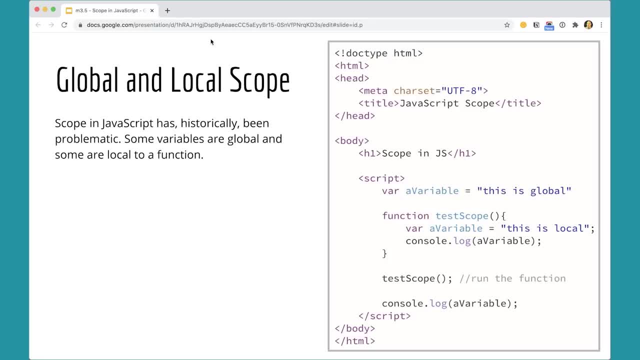 that were used on web pages to do some interactive things, and that was about it. They didn't expect JavaScript to become a general, all-purpose programming language at that point, So scope was not really very big of a concern, But JavaScript has become a general programming language. 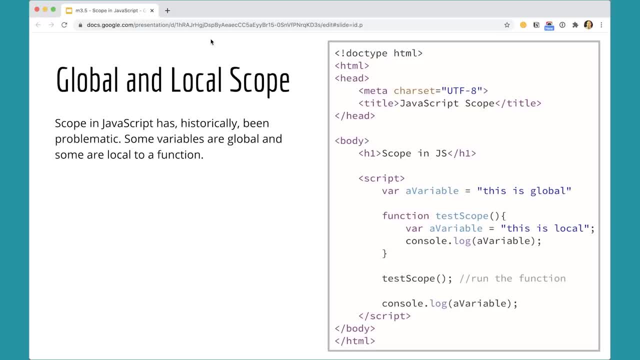 and scope is now a pretty big concern and we need to be careful about it, And this is another thing in the language that is potentially problematic and that you want to be really clear about and have some best practices around so you don't make mistakes and get unexpected results. 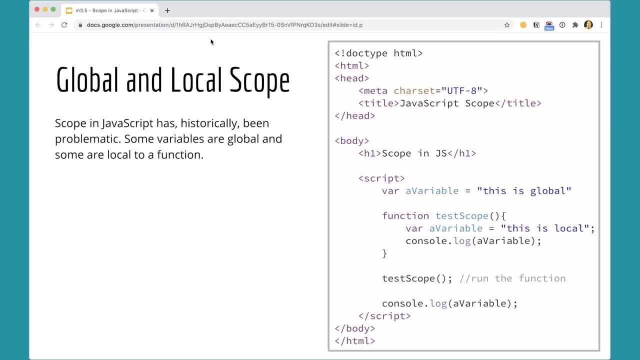 and spend a lot of time chasing down bugs in your code, because that's no fun. So let's talk about how scope works. If we look at this script over here- and I'm actually going to switch to my code editor over here because I have this written over here- 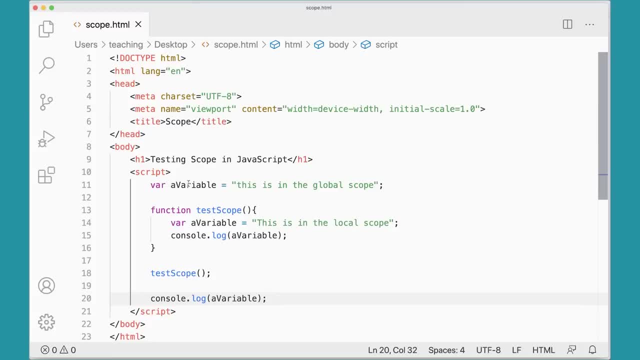 I have a variable called a variable and it's in the global scope. It's not defined. it's defined within the script tag, but it's not defined within the scope, It's not defined in any sort of function. And then I have a variable also called a variable. 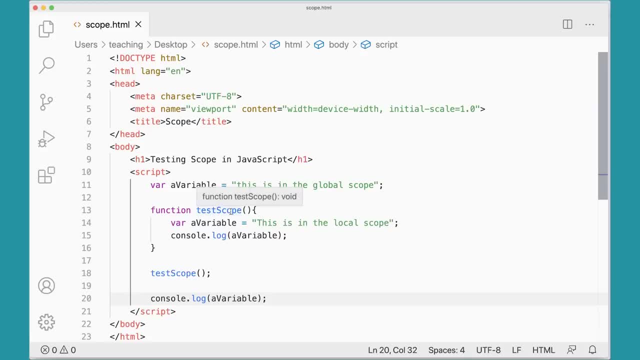 in the local scope And then I'm going to run test scope this function here which should print out this variable, And then I'm going to console log out a variable which should print out that variable. Let's see if that actually works. 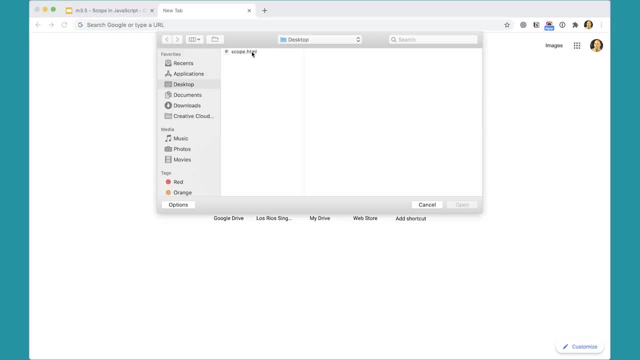 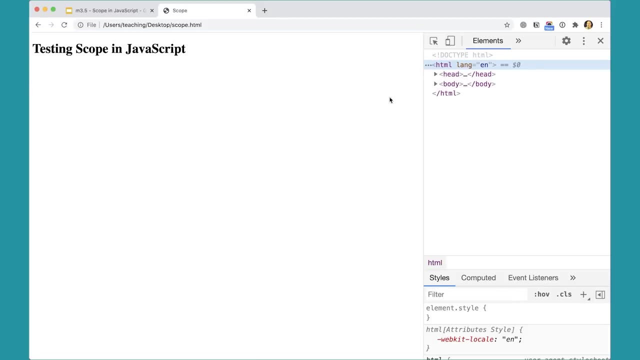 I'm going to open a new tab here and do control O and open up scope and click open And we get that and do inspect And I'm going to move this thing down to the bottom and click on console And you can see this is in the local scope. 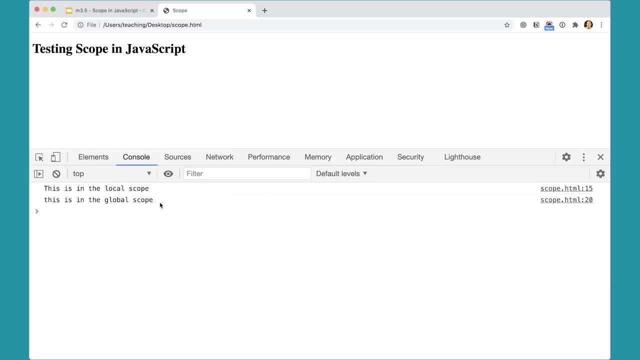 and this is in the global scope. So I have two variables with the same name with two different values, And that's kind of that. It's not really a great thing to have happen there, But you can do that kind of thing with JavaScript. 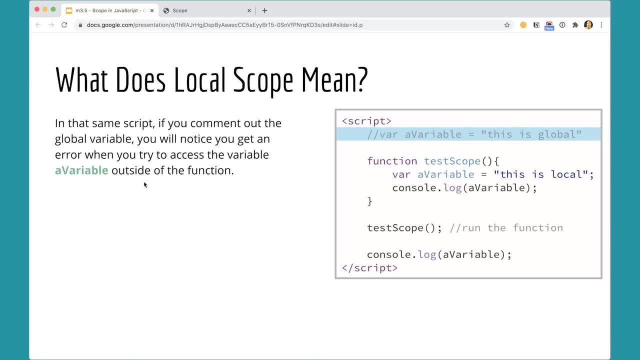 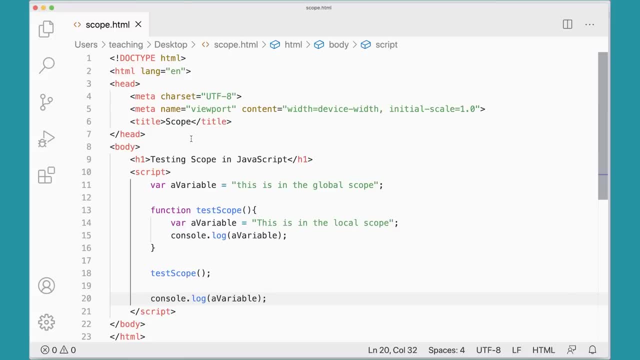 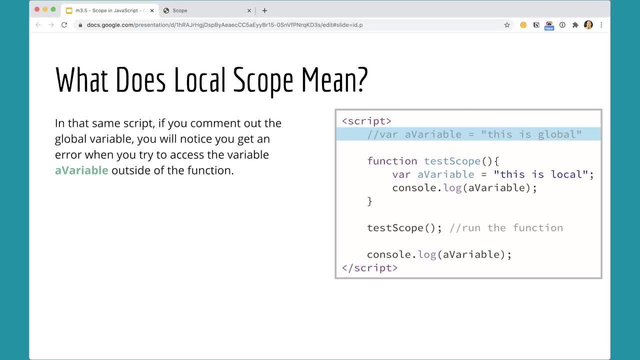 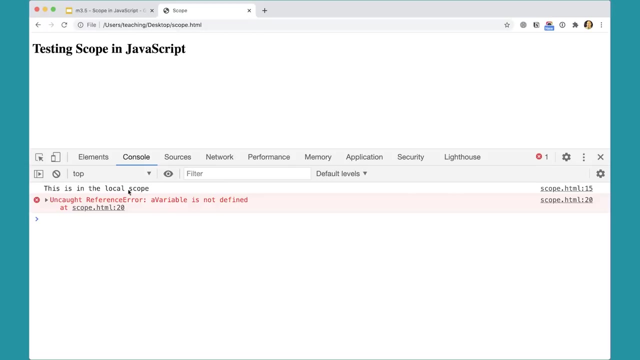 And it's not great. So what does local scope mean? Well, let's do this for a second. Let's go ahead and take this out of here and then run that file again. Now, this one's running because it's inside the local scope. 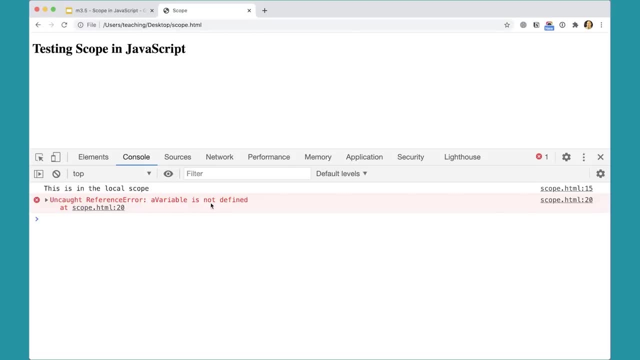 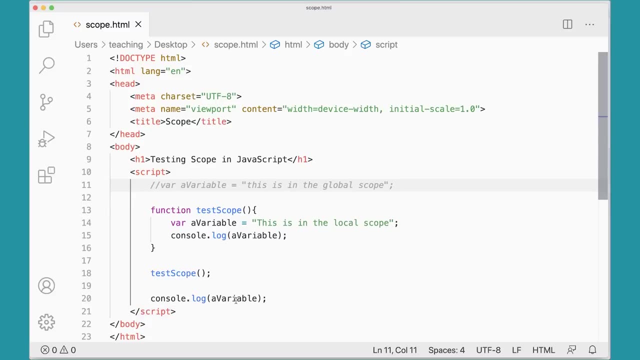 But the one that says a variable. this says a variable is not defined, Because what happens here is that I cannot access if this variable doesn't, a variable doesn't exist. I can't access this one from outside this function, because this variable is only accessible. 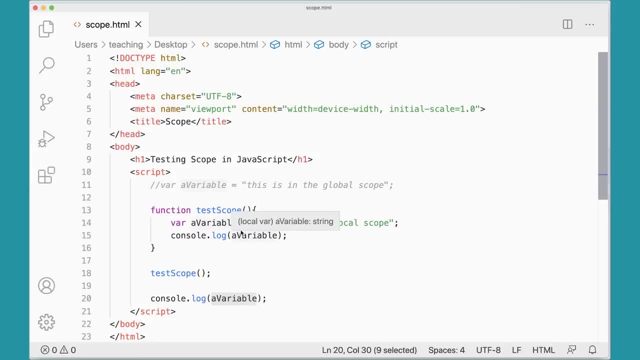 with inside the scope of this function, And so that's what local scope means- is that it's local to inside the function and I can't access it outside the function, And that can be very important for making sure that we don't have problems with variables. 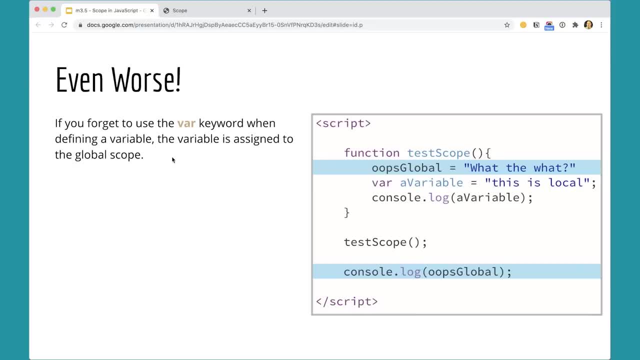 Okay, great, Even worse. this is what happens when things get even worse In JavaScript- and we've seen this before- is if I make a variable and I forget to use the var keyword, that variable automatically becomes part of the global scope. 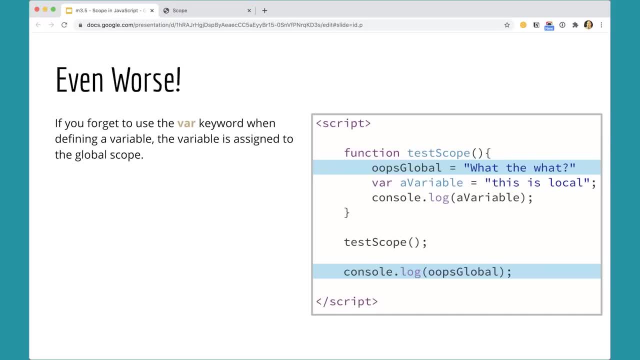 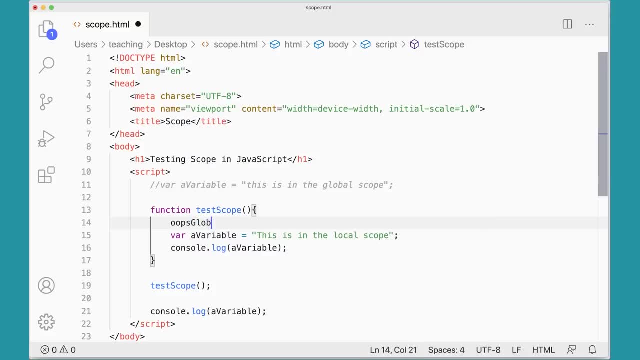 So I'm going to go ahead and add this in here and see what happens. I'm going to make another variable called oops global, but I'm not going to use the var keyword equals. this is accidentally global, And then down here you'll notice I can access that variable. 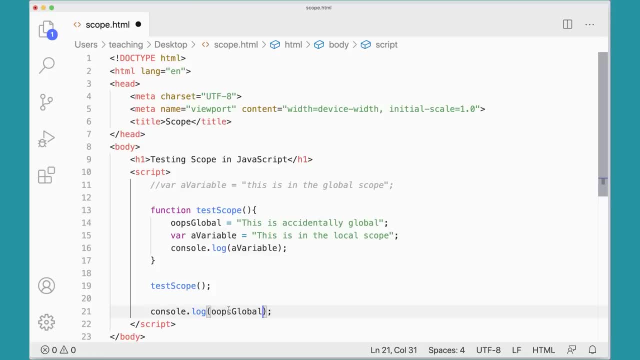 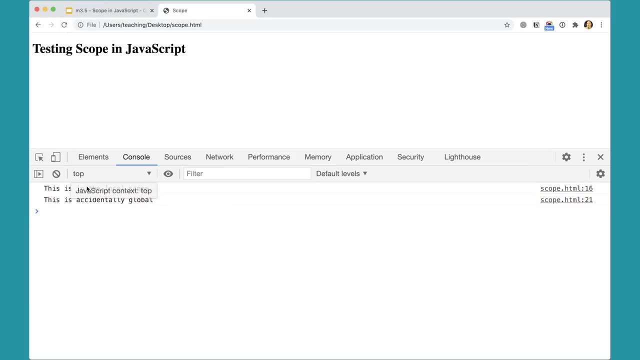 even though it's defined- kind of defined, because I didn't use the var keyword- it's not really defined inside the function. It belongs to the window. So now you'll notice when I run this over here. this one runs, So I couldn't access the local scope variable. 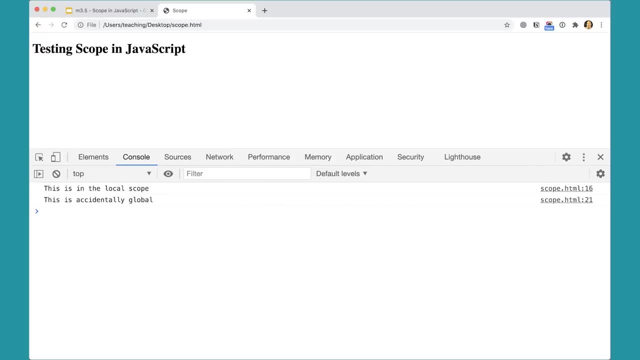 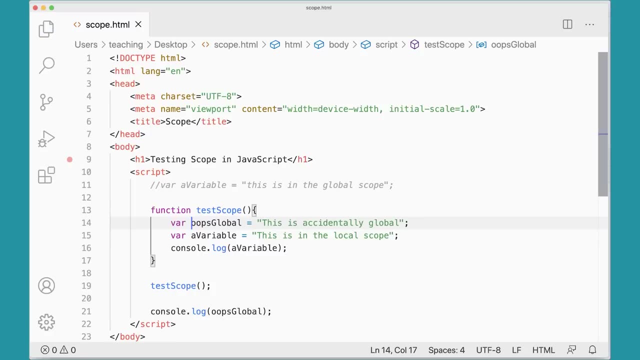 because it was inside the function, but because I forgot to use the var keyword here. if I put var in front of this, that will no longer be global and we'll get the function, That error happening again. So this is kind of a. 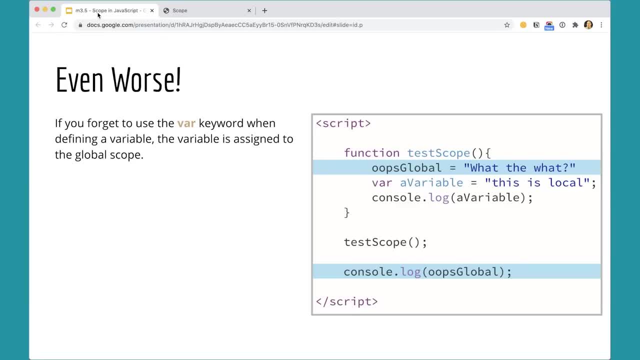 this is kind of a bad thing in JavaScript is that you could accidentally leave out var, just a keyword, and the variable will still be defined, but it'll be defined at the wrong scope level And that could lead to all kinds of problems. 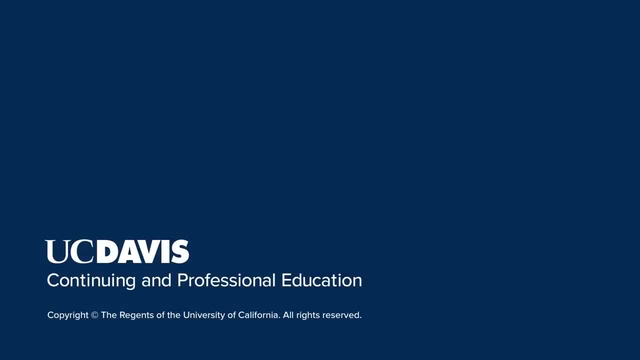 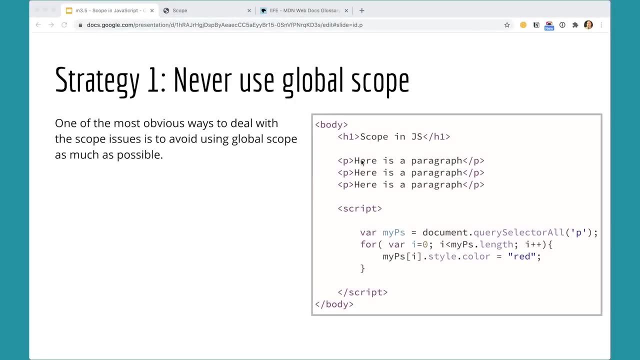 One strategy that we can use to deal with the global scope and trying to prevent problems there is to just never use the global scope whenever possible. So here you can see, I have a very simple script that is doing what we've done before. It's going in to our document. 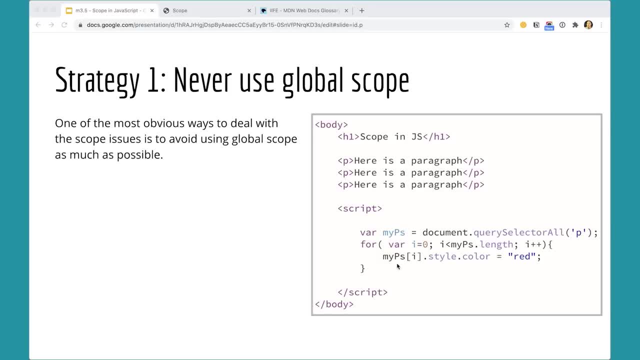 getting our paragraphs and then using a loop to change all the color for each paragraph to red in that loop, one at a time. It's going through looping that. But here my p's is in the global scope, The variable i is in the global scope. 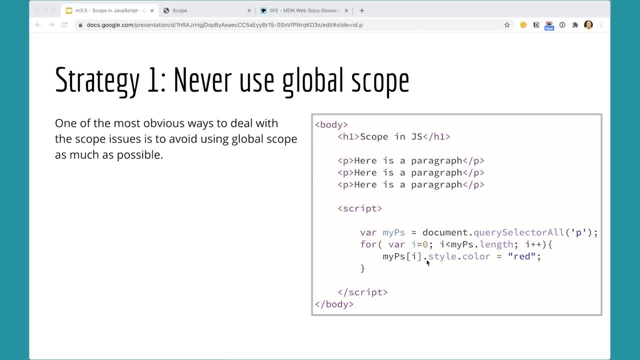 All of this stuff is in the global scope, So that could be problematic. So what can we do about that to keep it out of the global scope? One thing we can do is we can use what's called an IIP, An IIFE. 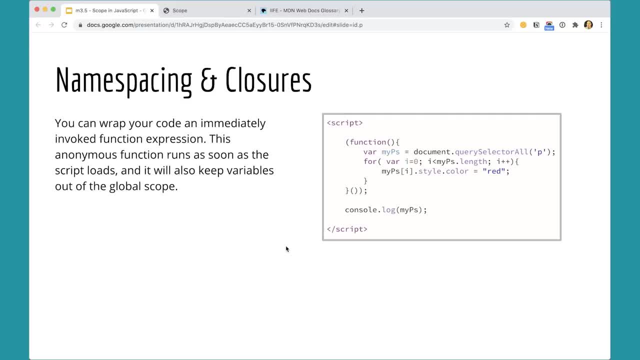 or an Immediately Invoked Function Expression. Basically, we wrap all of that stuff inside of a function that will just run automatically when the page loads. So we could take our entire, all our script and stick it inside of one of these sort of self-running functions. 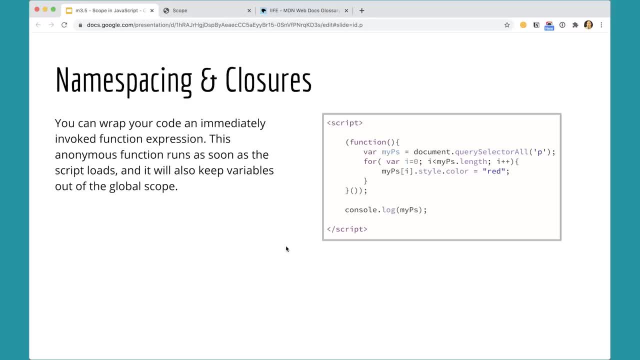 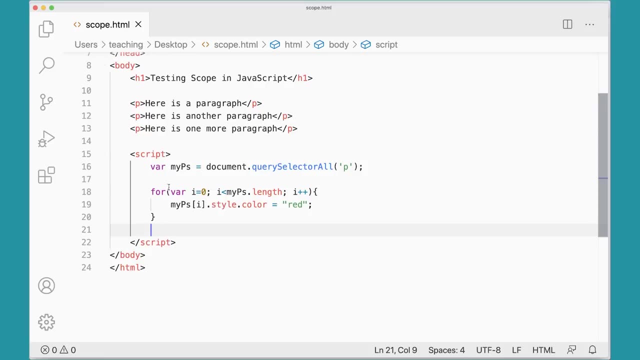 and it will just run and do its thing inside the function. It'll keep the variables local to that function. So let's take a look at how to do this really quickly. Over here I have my script and you can see that I'm getting my paragraphs. 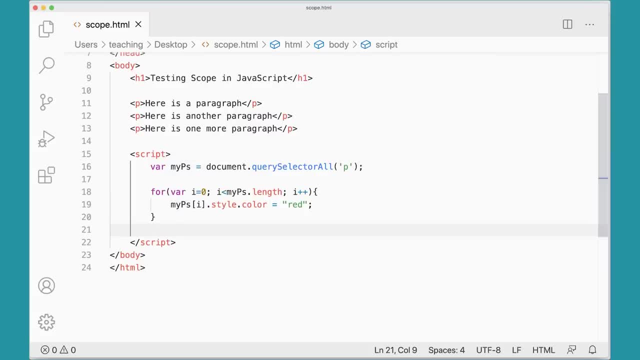 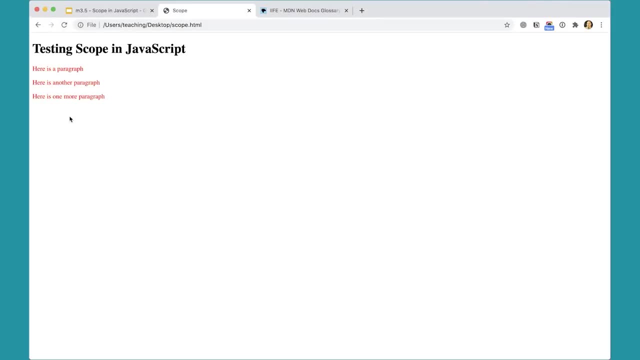 I've got my for loop here and it's going through and doing that kind of thing, And then if I come back here and actually run this thing, you can see that it's actually turning these paragraphs red. So that's all working. 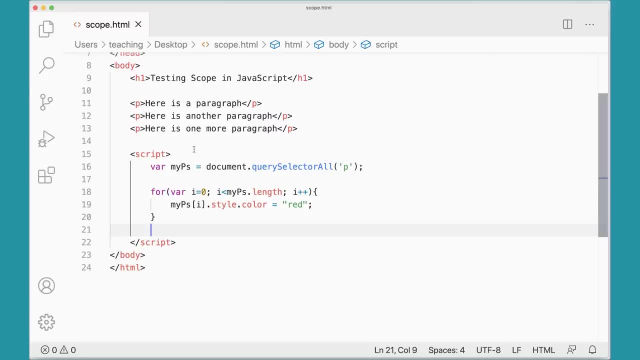 working as expected. The way to use the IIFE- the Immediately Invoked Function Expression- is like this: We type a set of parentheses and then inside the parentheses we put a function which has its own parentheses and its own curly braces. 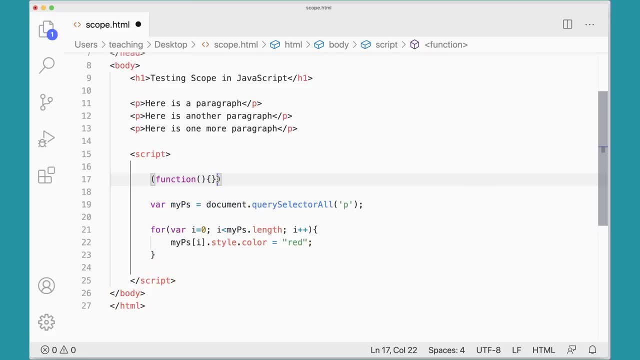 And then we add one more set of parentheses to to force it to run, And we can put a semicolon at the end of that, And then when we click in here, we can actually take this entire thing and stick it inside of that function. 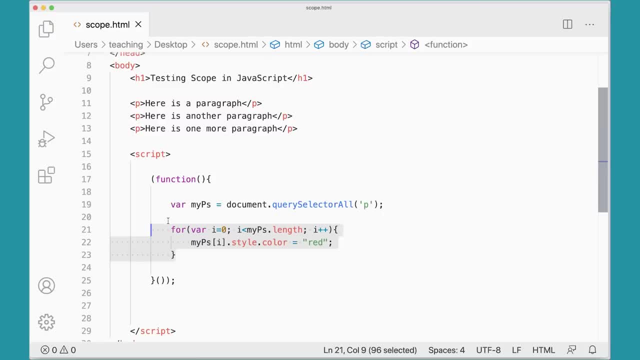 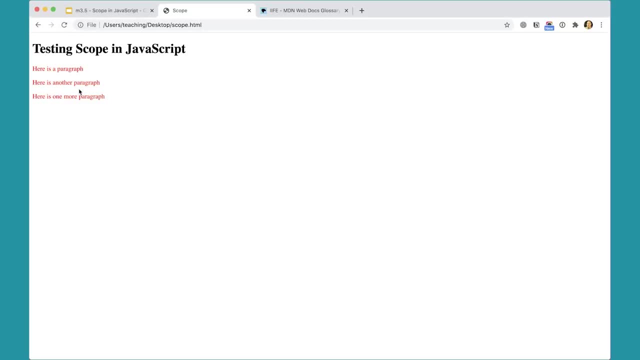 There we go, And now that function will run when the page loads. So if I come over and refresh it, you'll see it just runs and it works just the same as before. But what's different now is that these variables are now local to this function. 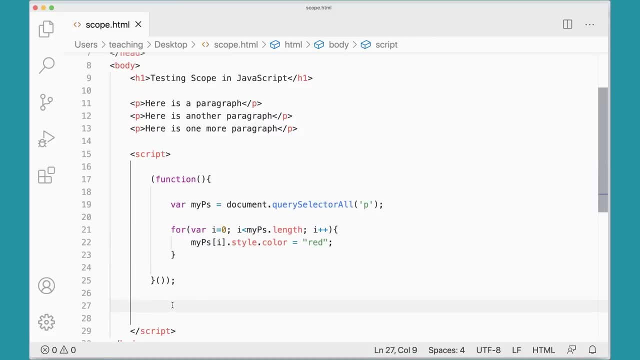 and they're not in the global space. So down here, if I do consolelog myps, I'm going to get an error, which is what I want. I want to make sure that I cannot access the variable myps in the global scope. 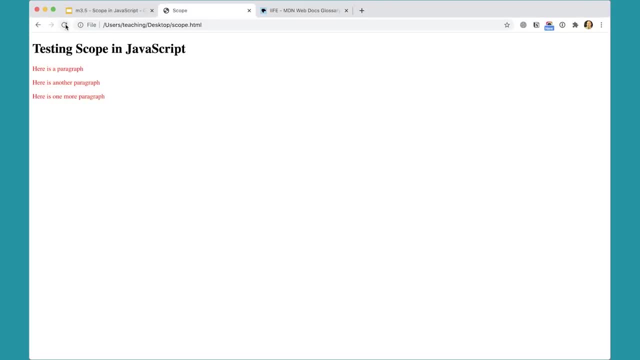 So if I do that and then come back over here and run this again, it'll run fine. But if I inspect you'll see in the console I'm getting an error. myps is not defined because it's not in the global scope. 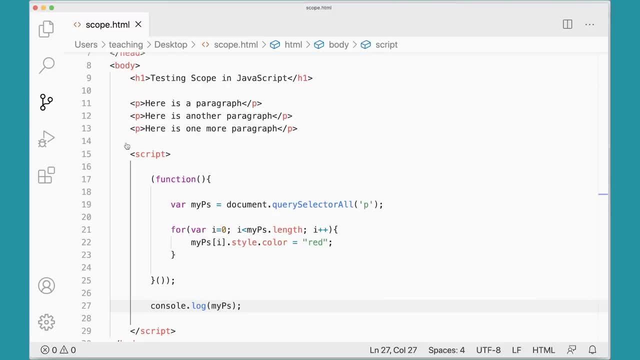 So, again, I'm going to do that one more time because the syntax is just terrible, But it really is helpful for making sure everything stays in the local scope there of this function. So I'm going to get rid of that again And I'll just do this one more time. 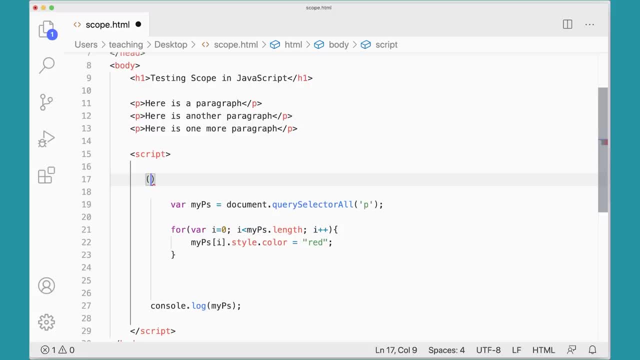 So we start with a pair of parentheses And in there we add a function with its parentheses and its curly braces, And then, to make it run immediately, we put another set of parentheses like that And we just put a semicolon at the end. 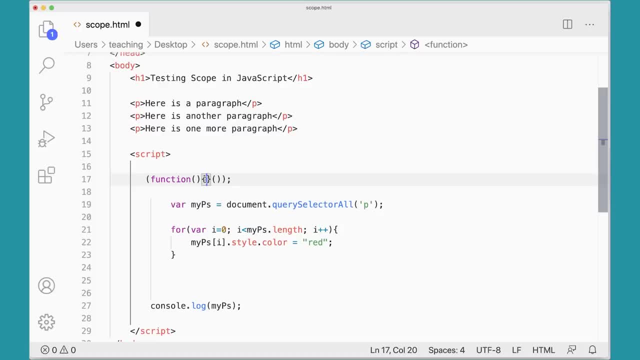 And then this is what's going to hold all our code. So we put that in between the curly braces, move that down, and then all of this stuff can just go inside here, Like so, And once you've typed this function expression a few times, 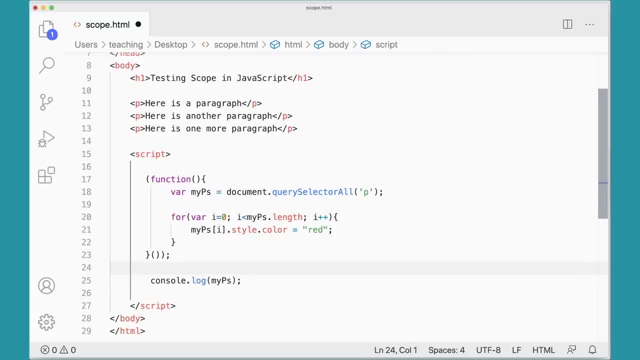 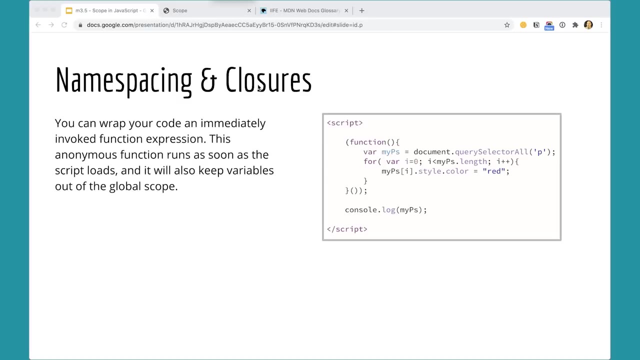 you'll get comfortable with it And then that will work just fine, And it keeps everything local to this function expression. There are a few more things that I want to say about this while we're here. This is also called namespacing, because we are making sure. 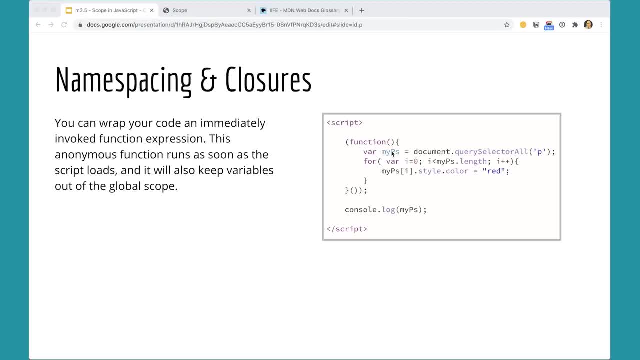 that the space for the name for this variable is set so that it's within this function. So that's actually a namespacing thing, And namespacing has to do with where things are available. Another thing to point out is that any function in JavaScript. 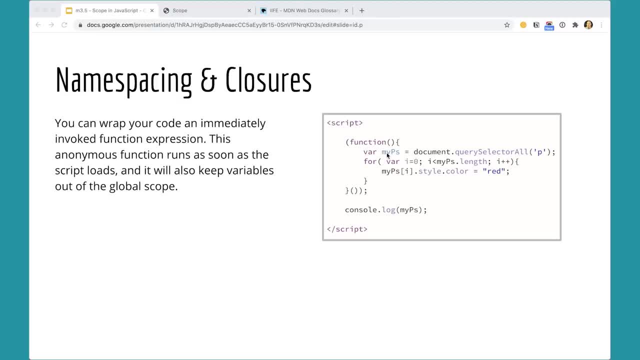 is a closure. really All functions are closures. Anything that you put inside of a function is going to keep those variables from creeping out into the global scope, unless you forget the bar keyword, And we'll get to a fix for that in a minute. 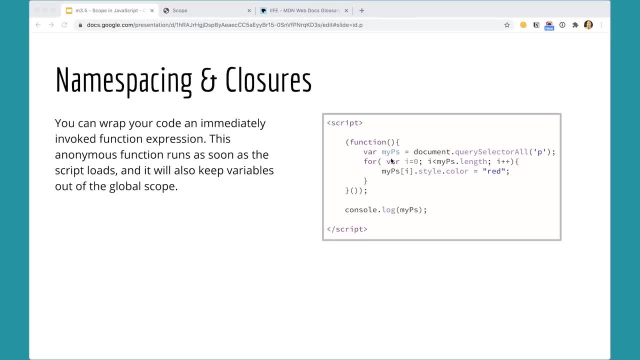 But that's an important thing And often when we talk about closures in JavaScript- if you look it up on YouTube, closures in JavaScript- although technically any function is a closure- really what people are talking about. usually when they're talking about closures. 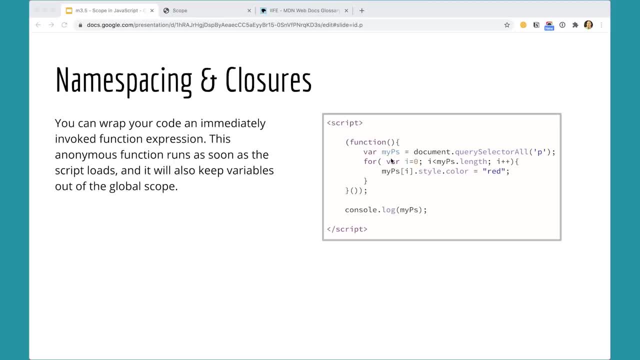 is not just keeping the variables local to the function, but also being able to get data out of those closures as well, And we're not talking about that part at this point. We'll deal with that in a more advanced course, But here we're just looking at. 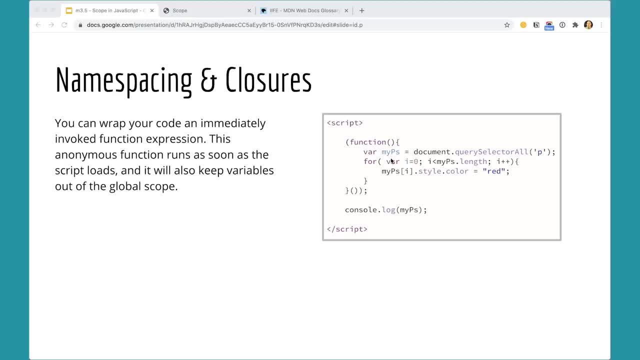 how do we keep the variables inside the closure for this particular, for this particular function? How do we keep it inside there so that it doesn't pollute the global scope? And that's the terminology that we use: polluting the global scope- And one of the reasons why we don't want to. 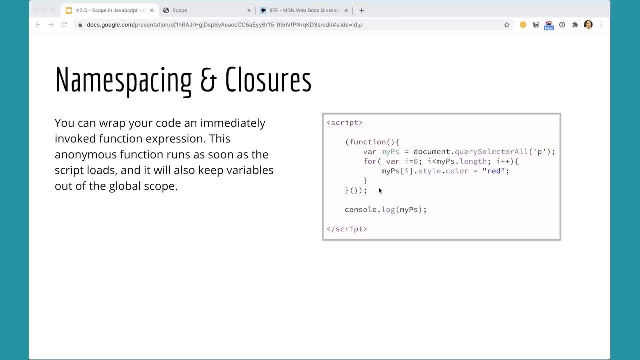 pollute. the global scope is we could be combining scripts from other people And they could have variables with the same names And these variables could collide with each other And you could get unexpected results, because you think a variable is holding one value, but in fact it's holding another. 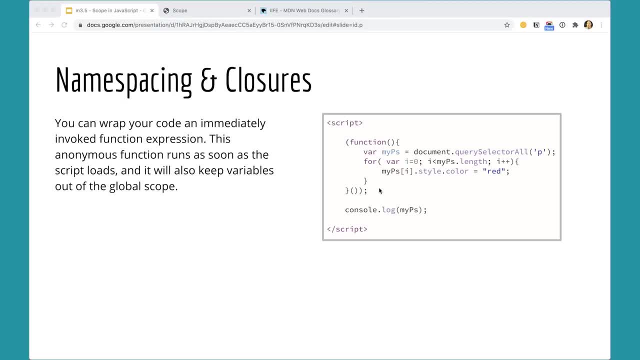 because it's coming from another script, because they didn't keep their variable values local And they let them creep into the global scope. Those are some of the problems that you can run into with more complex scripts. So there's that. One last thing I want to go over really quickly here. 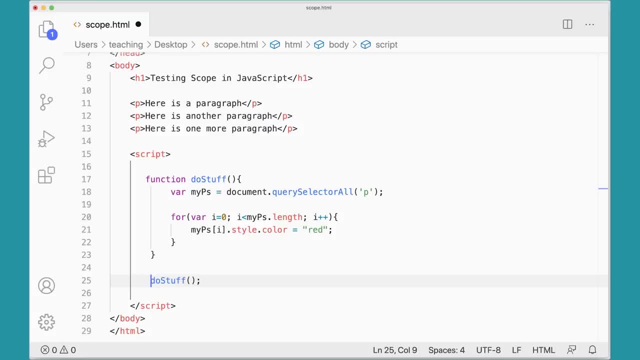 about the immediately invoked function. We can make a function here. I have my doStuff function back again And I can call it this way with doStuff, But any function can be immediately invoked. So if I comment out doStuff here, that's not going to do anything. 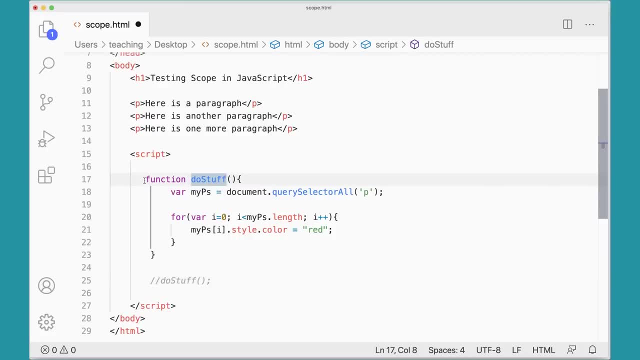 It's just going to define the function, But I could put a parenthesis in front of this and a parenthesis at the end of it, And then a set of parenthesis and semicolon, And now that function will run. doStuff will run right off the bat. 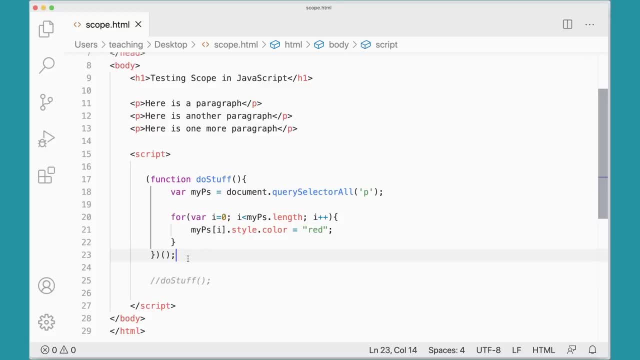 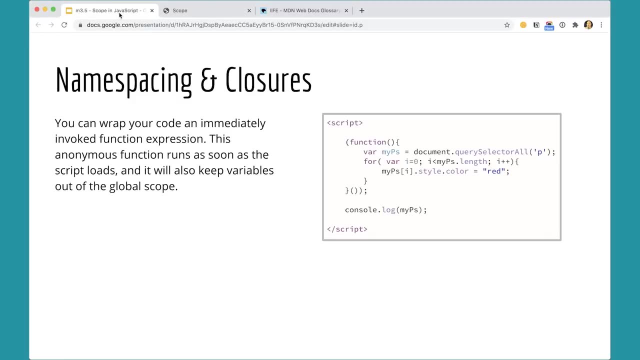 without having to actually call it like this. So this is an immediately invoked function as well. So if I do that and then come over here, save that and then come over here and test it, you'll see it runs just fine and it does everything it needs to do. 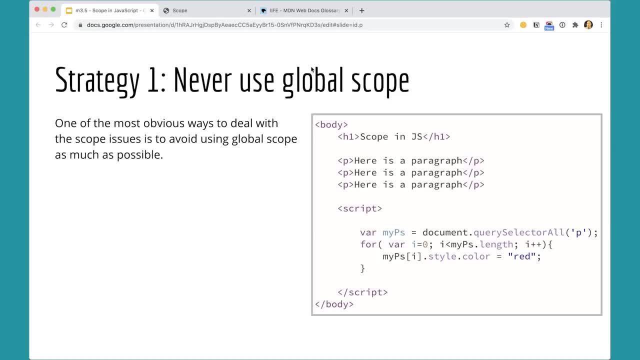 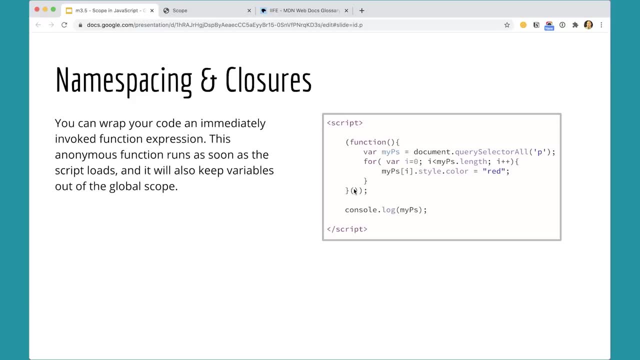 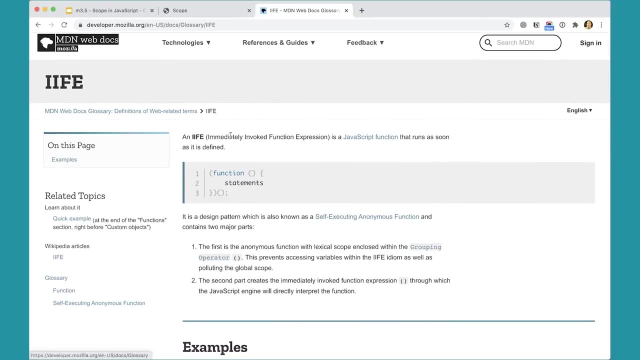 However, we're using the anonymous function here, this anonymous function here just as an anonymous function that will just automatically run, And I have that page open over here in the MDN for the IIFE, the Immediately Involved Function Expression, which will explain more about. 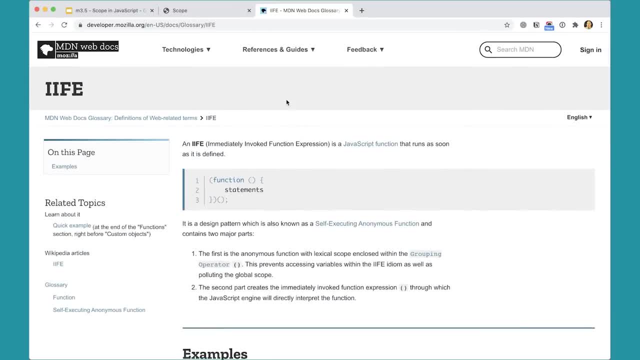 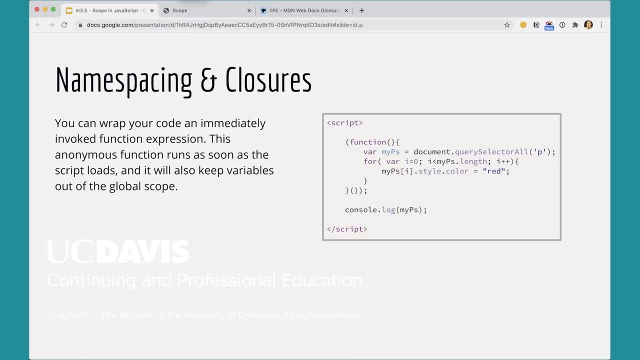 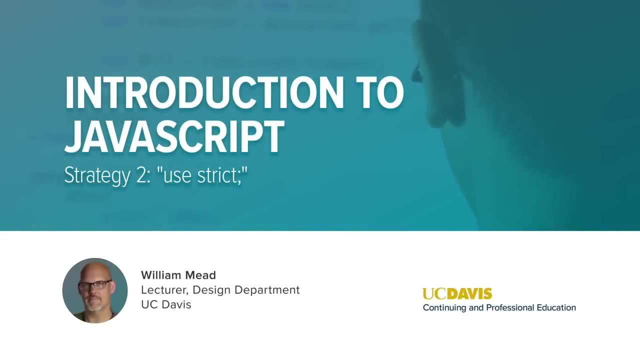 how this works and what it does. It's kind of a useful technique that we have at our disposal. Okay, great, We'll look at the next thing in the next video. The first strategy was to use some sort of closure with namespacing. 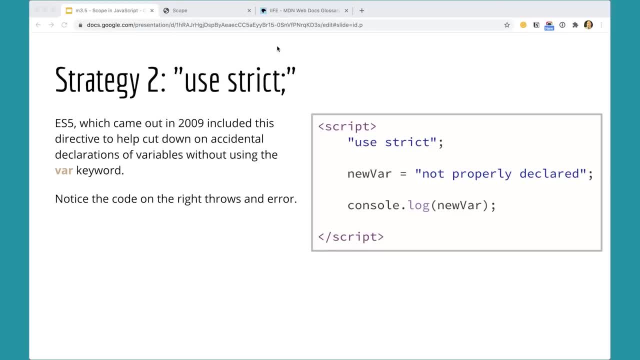 to make sure that variables stay out of the global scope. The second strategy is to use this useStrict directive, And this is something that came out as part of ES5, which again came out in 2009,, because it was recognized fairly early on. 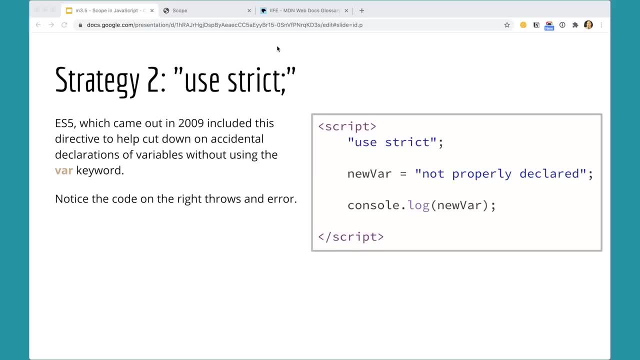 that the issue of forgetting to use the var keyword when defining a new variable is really very problematic, or potentially very problematic. So we want to have that not happen And let's take a look at how this works, because this is kind of interesting. 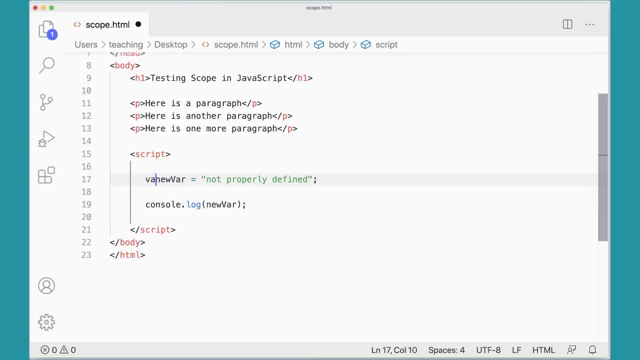 So over here I have a variable and I didn't put var here like that, So I've left off the keyword. So this new var is going to get defined in the global scope, And it is in the global scope anyway because it's not inside of the function. 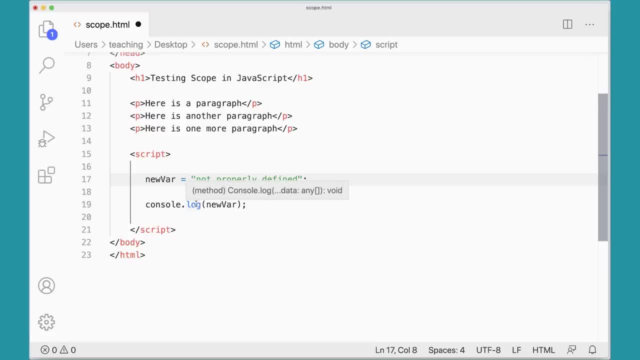 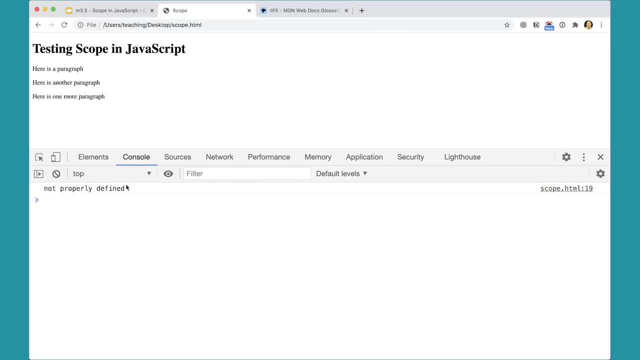 But that's OK, We can do this And we can console log that out And I can save that and go over and run it over here in my browser And you'll see that that variable gets sent out to the console log as described there. 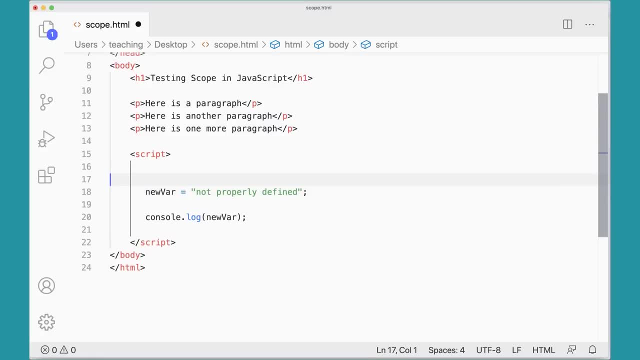 which is fine. But if I add the useStrict directive in here, useStrict like so and this is a directive, So we put that in there And then watch what happens. I come over and try to run this script again. 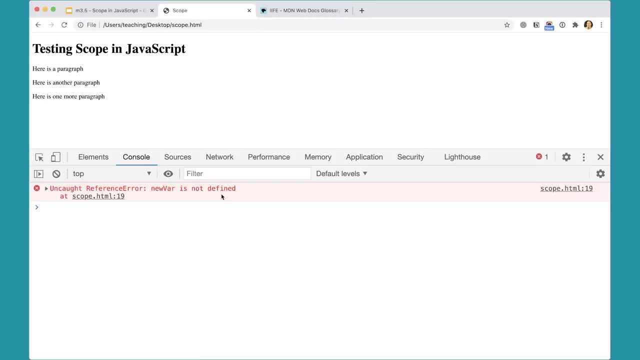 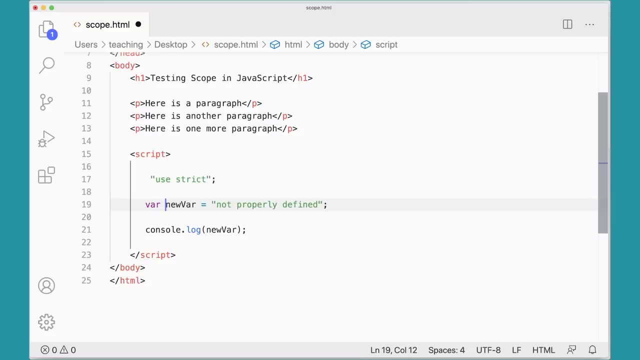 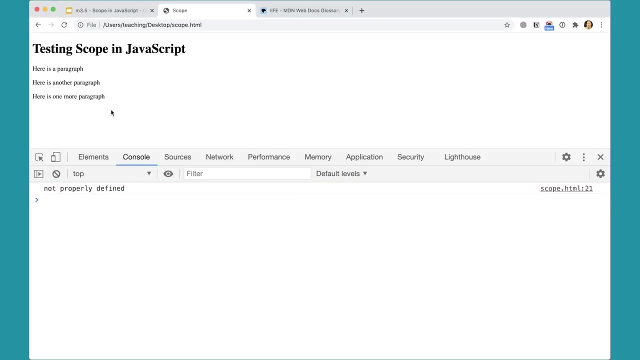 Uncut reference error. New var is not defined, So useStrict will keep me from accidentally forgetting the var keyword. If I put that in, it'll work just fine. There we go Now again. this is something that came out as part of ES6, ES5 back in 2009.. 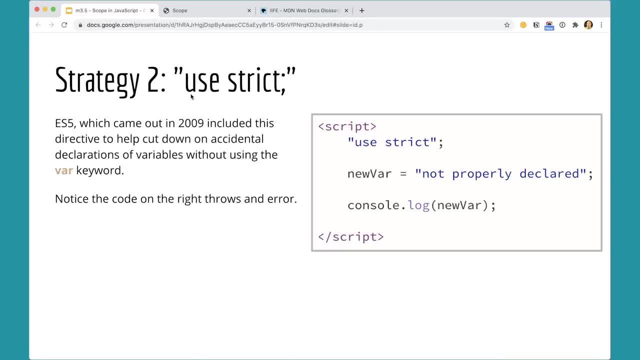 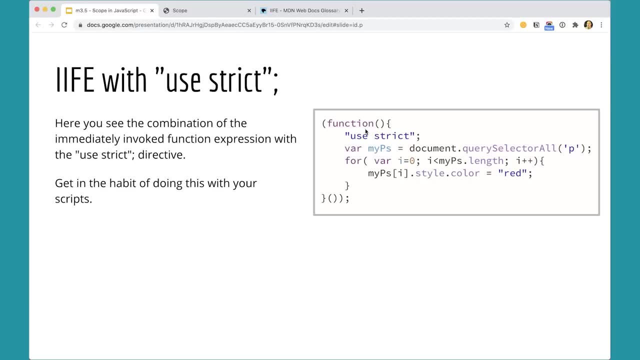 And that's kind of a very interesting and useful tool to keep us from doing this. And if we combine these two things together, the IIFE or the closure, if we make sure that everything is enclosed inside of a function and the useStrict directive. 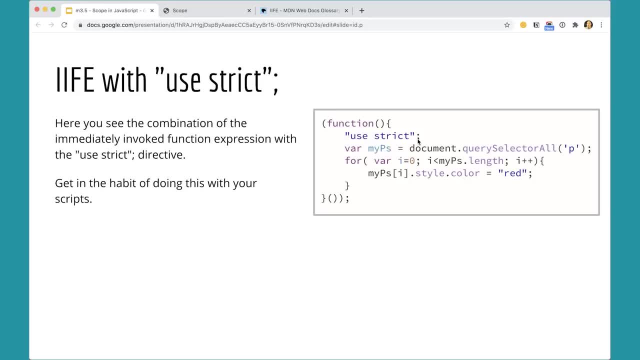 if we do those two things together, we'll be making really big progress towards making sure that our variables are staying within the proper scope for our functions and everything. So that's really great. And as you go forward with working with scripts, I strongly recommend. 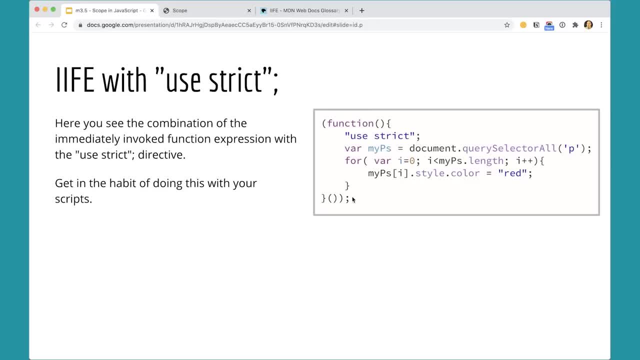 that you use both of these two things, And I'm going to give you sort of an exercise that will help you with practicing this in just a few minutes. I just want to show you one more strategy that's going to help us with scope. before we do that, 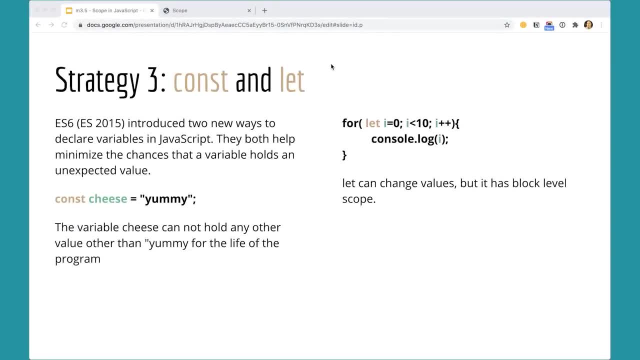 The third strategy that will help us with keeping track of scope is to use const and let as keywords for defining variables instead of var. So const and let were added introduced into the language. They were added to the language as part of ES6 or ES2015.. 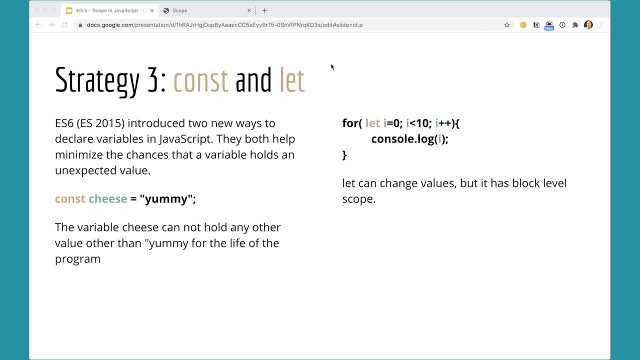 And they both help to minimize the chances that a variable holds an unexpected value. Const will hold a value, but once you've set the value for a variable, you cannot change the value of that variable while the script runs, So that will keep you. 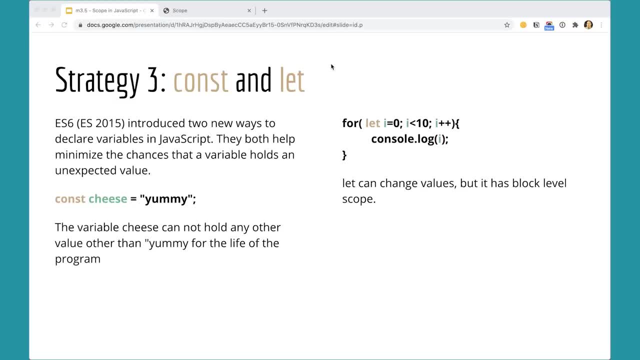 from accidentally reassigning a value to a variable that has been defined using the const keyword. So here I've got: const cheese equals yummy. And now that that's been set, while the script runs it cannot be changed. The let keyword allows you to change the variable. 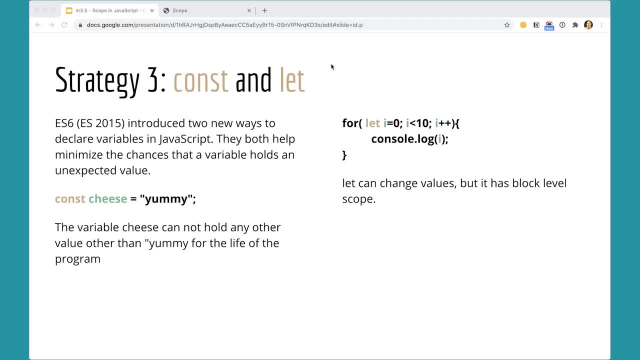 but it has block level scope. So here let i equals zero, that i is only available as a variable inside this for block, this for loop block, And it won't be available outside of the for loop block. So that adds a third level of scope. 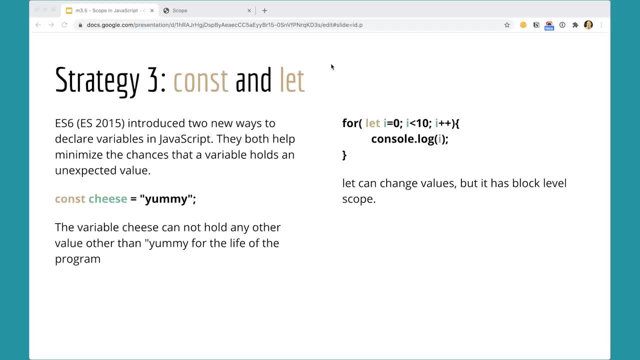 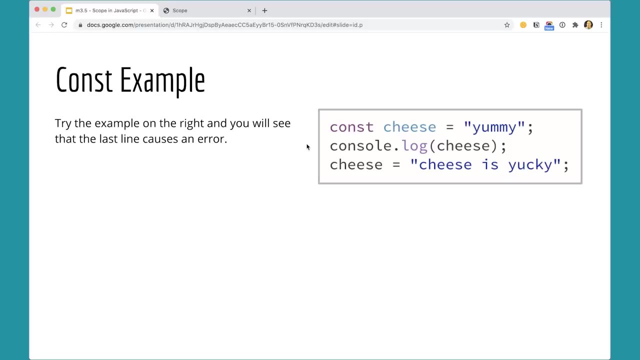 to JavaScript. Previously we had the global scope and we had scope inside functions, but we didn't have any block level scope. Now we've got a block level scope. Let's take a look at a couple of these examples. First, let's look at const. 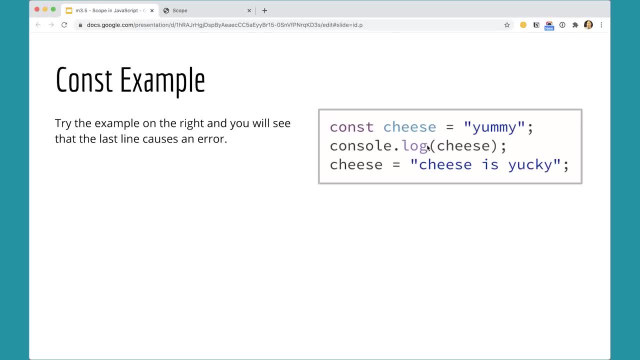 So here I have: cheese equals yummy and I can console log that out. But if I try to assign a different value to cheese I'm going to get an error. Let's just see, I have that over here in my code editor here. 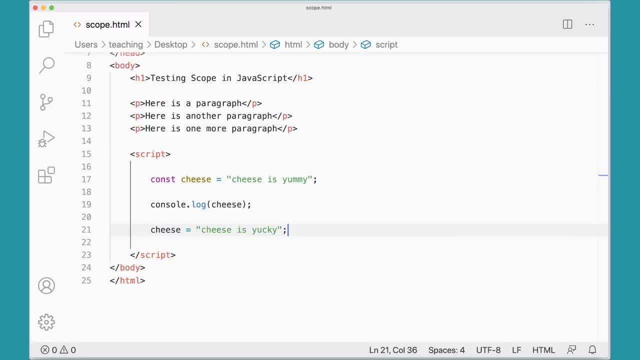 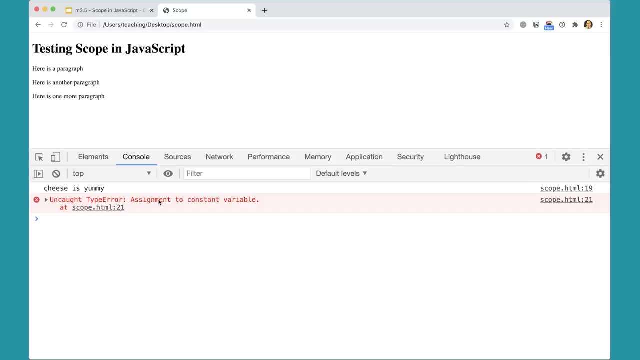 And that's great. So we can try to run that and see what we get. When I run that over here, what I get is uncut type error. assignment to constant variable. Cheese is yummy ran. That ran fine, but I could not assign a new value. 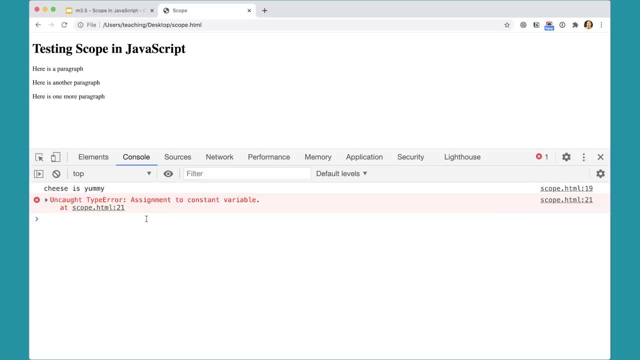 to that variable without getting an error, And that's going to keep me from accidentally assigning a new value to that variable when I don't want to or I want to make sure it doesn't change. So that's going to keep me from getting an error. 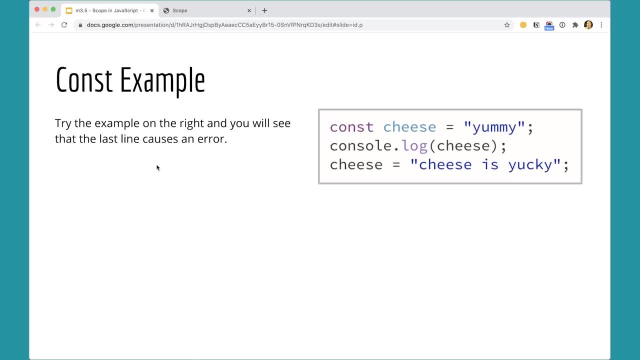 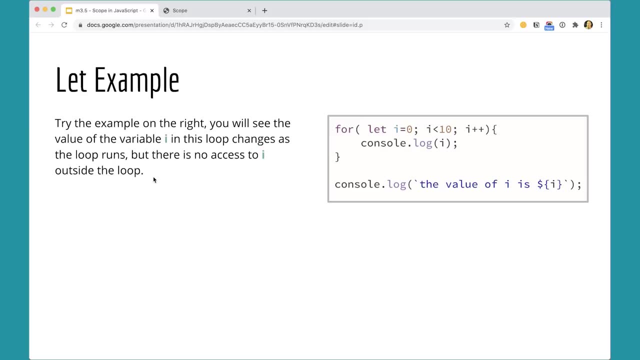 That's going to really help. The next thing we can look at is the let keyword and using that instead of var. We'll do this with a for loop, So let's go over to our code editor and put this one in really quickly. 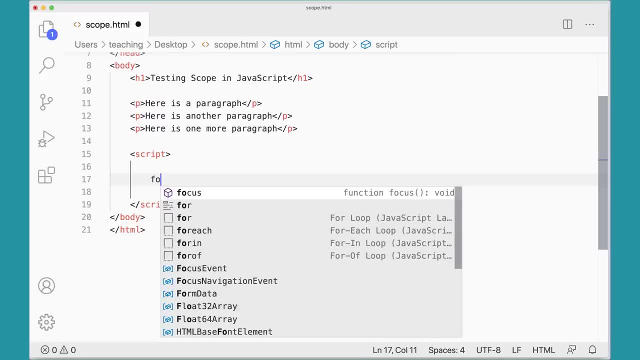 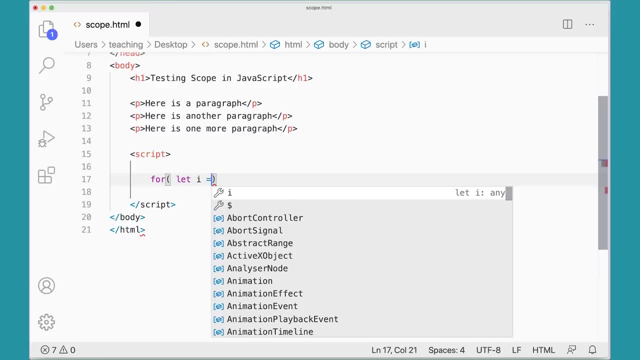 I'm going to just make a quick for loop here for And instead of using var, I'm going to use let I equals zero. Zero, not O. Let I equals zero While I is less than 10, something like that. 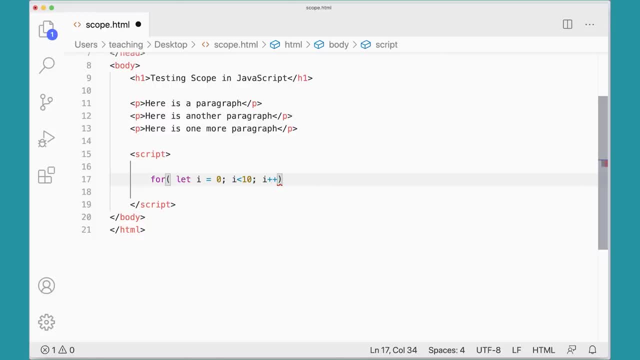 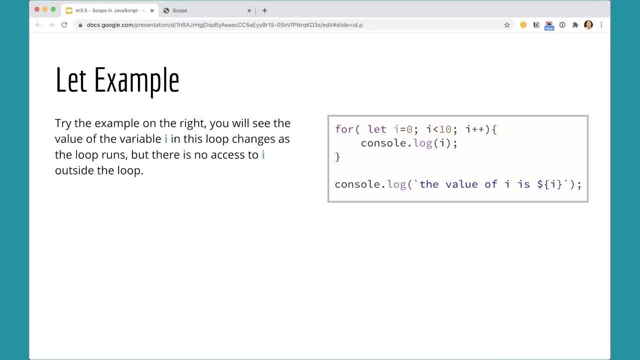 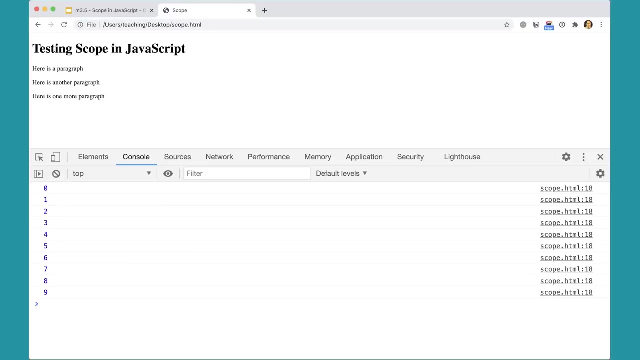 There we go, I plus plus, And then curly braces, console dot log I. And if I test this, you'll see that I will get printed out 10 times. That's as expected. So that's working just the same way as, let I mean as var. 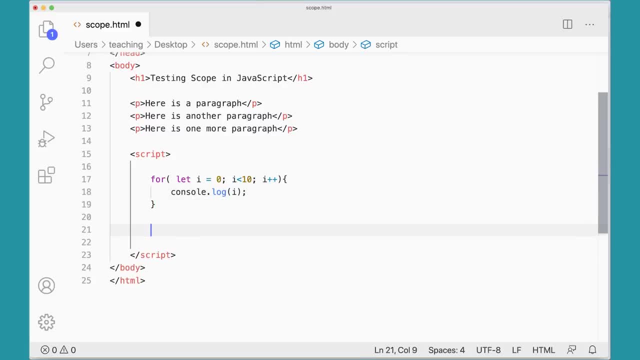 But if I come back here, if I try to do console dot log, use my tick marks. the value of I is I, But make that a variable Dollar sign. curly brace, Curly brace. That's going to generate an error. 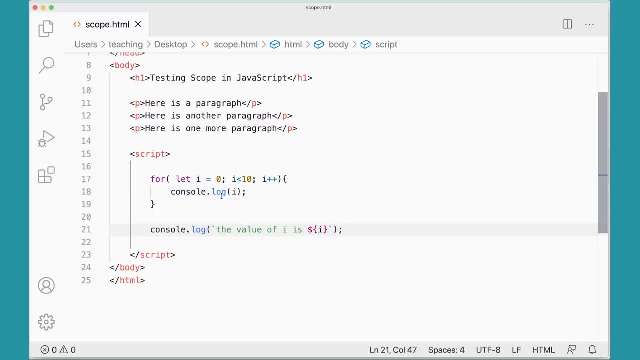 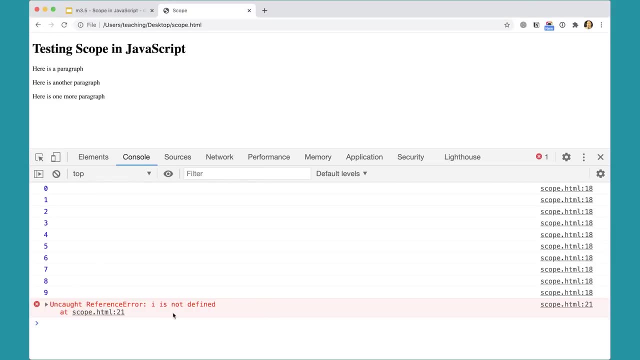 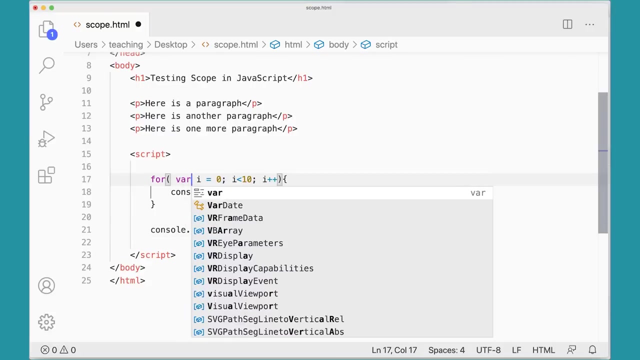 because I've used the let keyword and this has block level scope. Let's see that in action, I is not defined, Whereas if I were to come back here and change this keyword to var, that doesn't have block level scope. So if I save that, 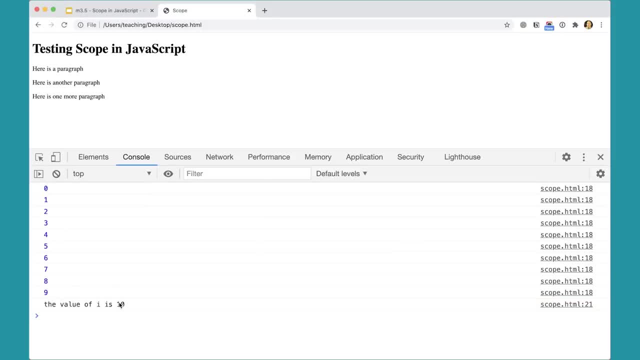 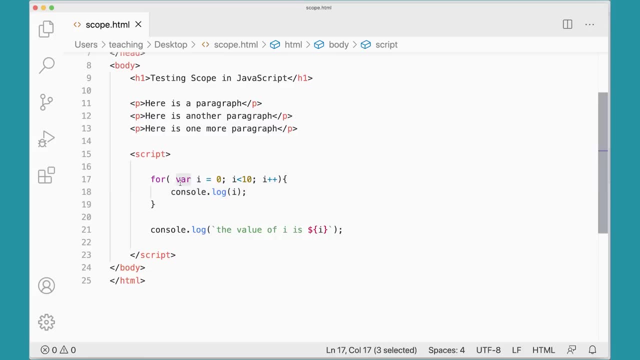 the value of I is 10 because it's gone through the whole loop and got up to 10.. So with var we don't have block level scope, but with let we do So with our third strategy. here, what we should do is: 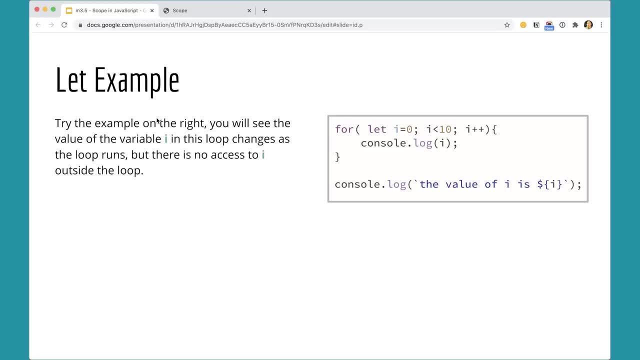 never use var to define variables anymore. Instead, we can use const or let And, in general, use const whenever you can Use const by default And then, if you actually have to have a variable, change values like you will in a loop. 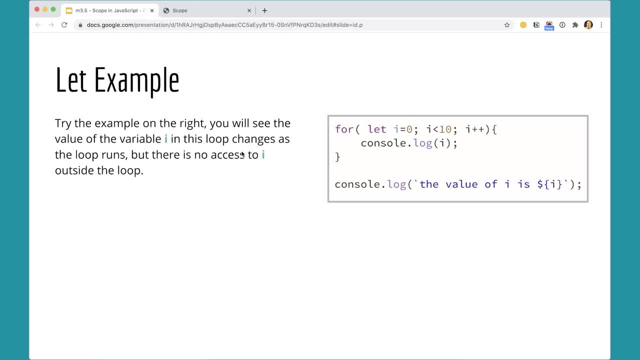 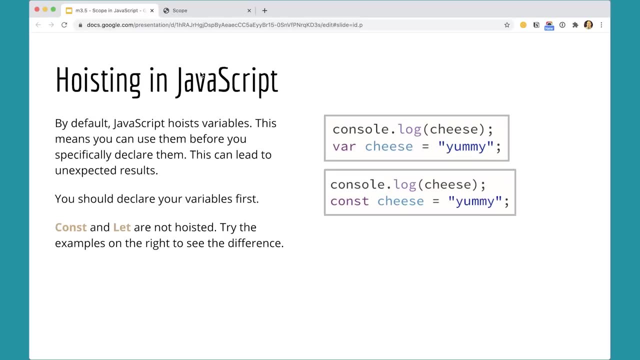 then you can use let, But mostly stick with const as much as possible. One last thing I want to talk about before we're done with talking about scope is hoisting in JavaScript, And this has to do with where variables and functions are defined. 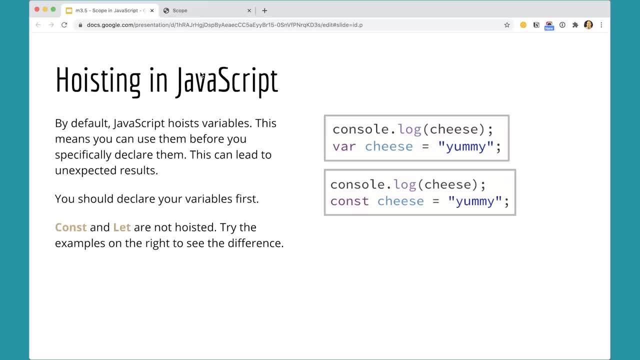 Generally speaking, functions and variables get hoisted in JavaScript, meaning JavaScript looks at the file and it sees that variables have been used, so it hoists them up to the top as well, as functions as well get hoisted up to the top. 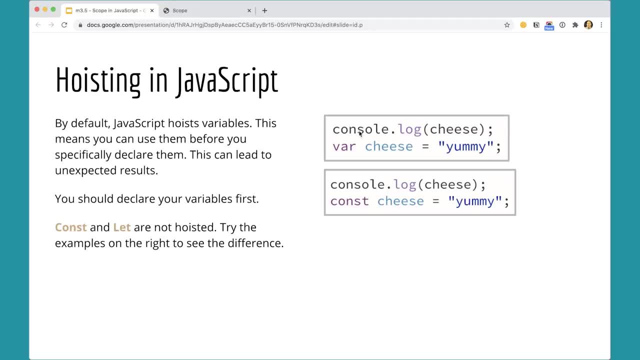 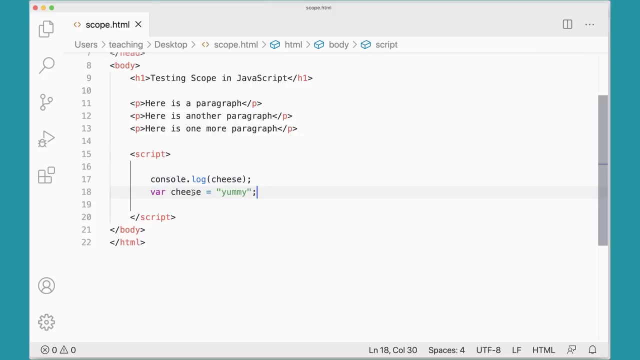 Let's see an example of this really quickly. So, for example, if I use the var keyword to define cheese but I console log cheese out, first, see what happens. So over here in my code editor I have console log cheese and then I'm defining the variable. 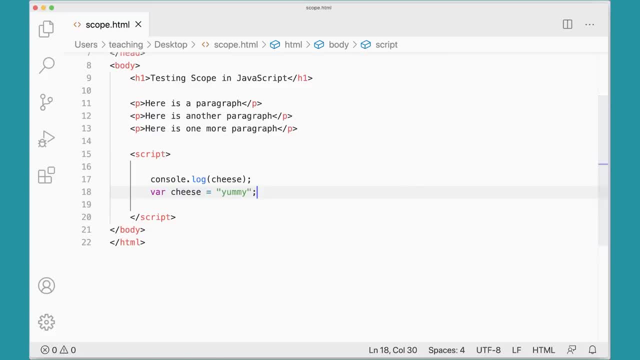 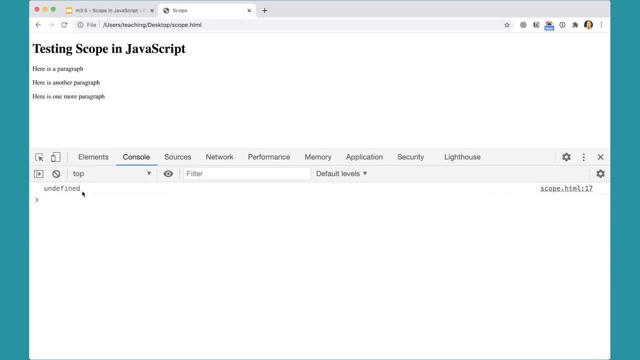 after I'm trying to run it in console. Notice what I get over here. If I refresh this page I get undefined, because the variable has not been defined at the point at which I'm using it. but it knows it exists because of the hoisting. 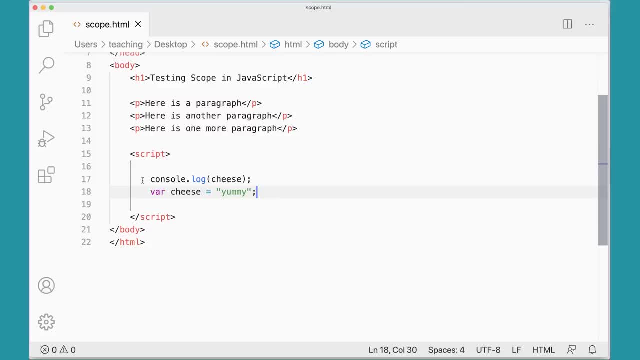 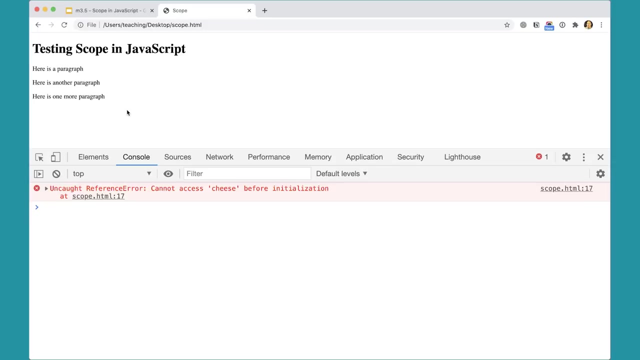 Whereas if I change that variable declaration there to const, watch what happens Now I get an error. And you may be thinking, why would I want an error? Well, really, what we're trying to avoid is unexpected results, And if you can explicitly get an error, 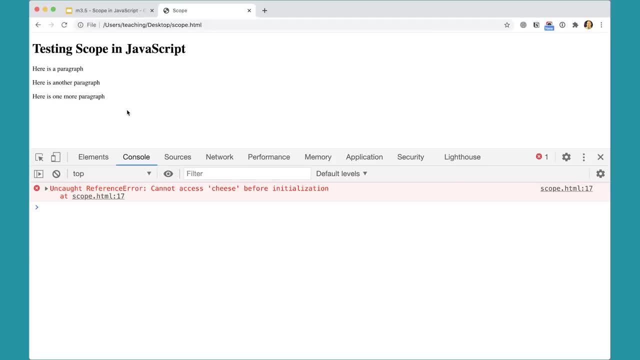 that says that it didn't get called right, then that's better than getting something that's undefined or something that's unexpected. So in this case, even though we don't really want errors, it helps us identify problems in our scripts before they become big problems and bugs. 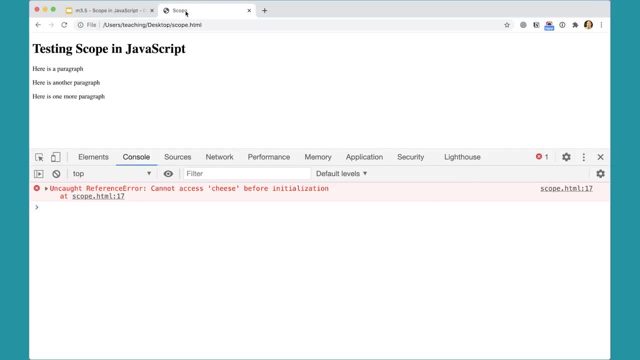 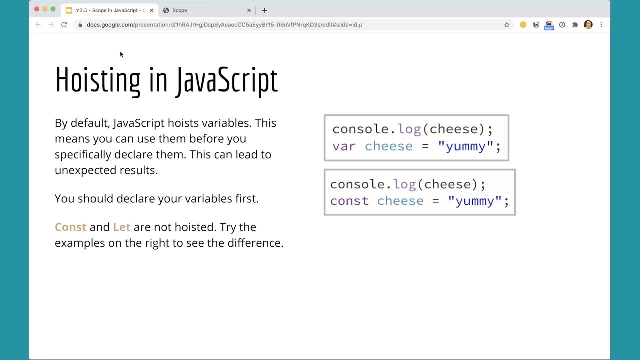 that are difficult to track down. Great, So with that, you've learned a lot about the scope in JavaScript and the different strategies that you can use. So let's talk about some of the things for dealing with scope in JavaScript, And they include: 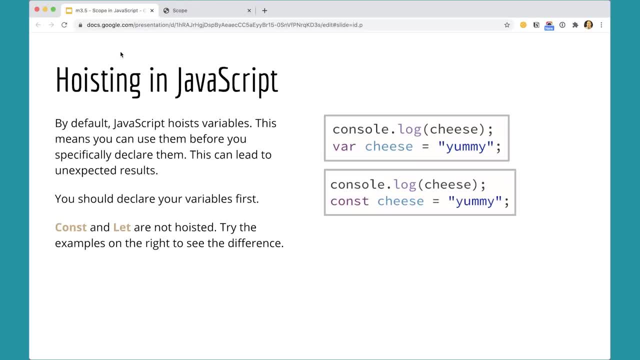 first and foremost, using some sort of closure or namespacing with the immediately invoked function expression to keep variables out of the global scope. That's number one. Number two: use the use strict declaration to do that and keep that going. And then number three. 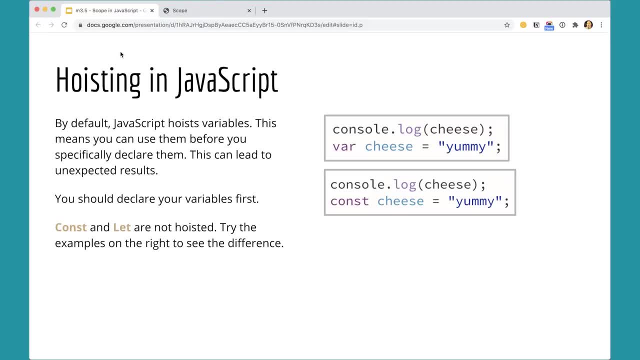 or the use strict to keep us from having variables that are accidentally declared without using the var keyword or any keyword from going into the global scope. And then, number three, use const and let as keywords to define variables. Those three strategies together will really help with making sure your scripts. 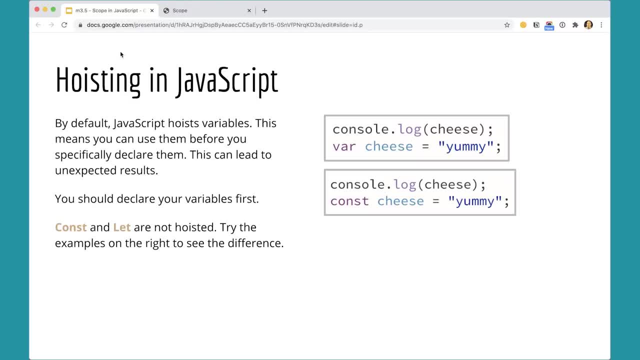 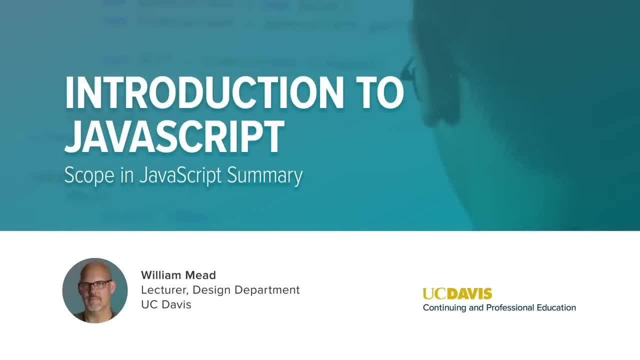 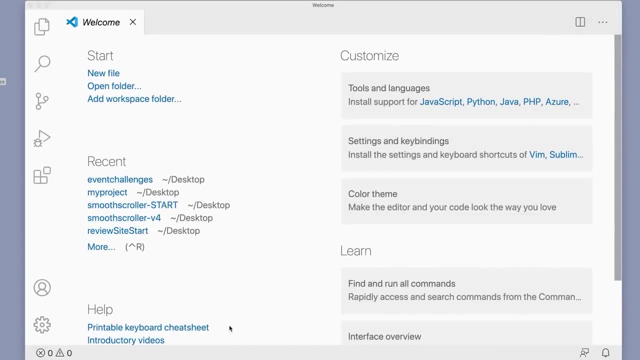 are more bulletproof and less prone to bugs and mistakes. The scope techniques that we just discussed take some getting used to, So I really strongly recommend you do this exercise to help you get used to them and get comfortable with them. Previously you had done some event challenges. 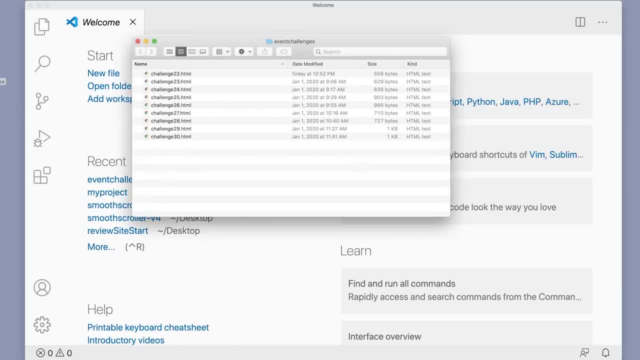 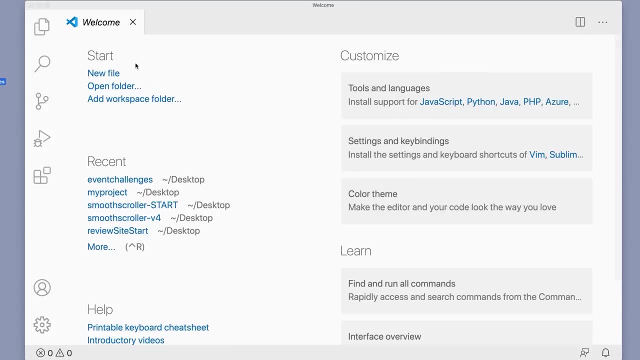 and I have that folder over here. So I have a folder here with challenges 22 through 30, and hopefully you have those as well- with all the completed challenges. If you don't, you should go do those challenges first. Then I have my code editor here. 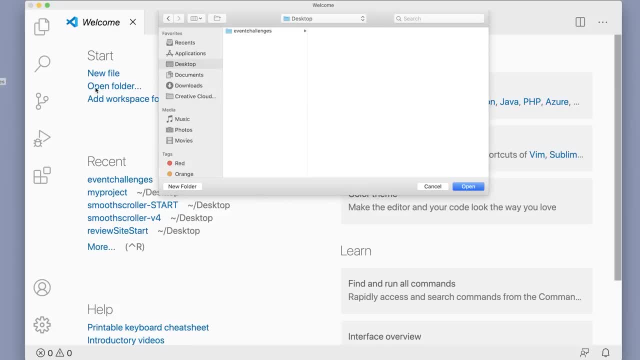 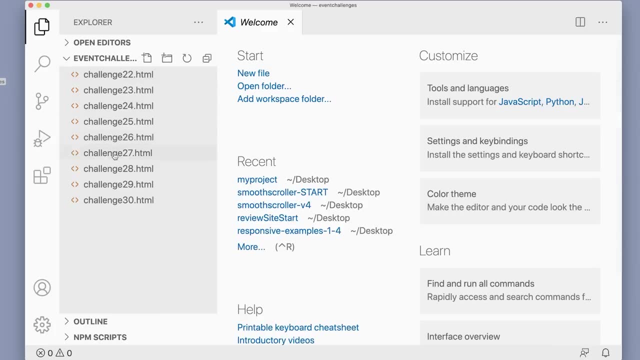 I'm going to open that folder in my code editor. by clicking open folder, I can open my event challenges folder here and it will show up on the side over here, So that's great. Next, what I'm going to do is practice these best practices. 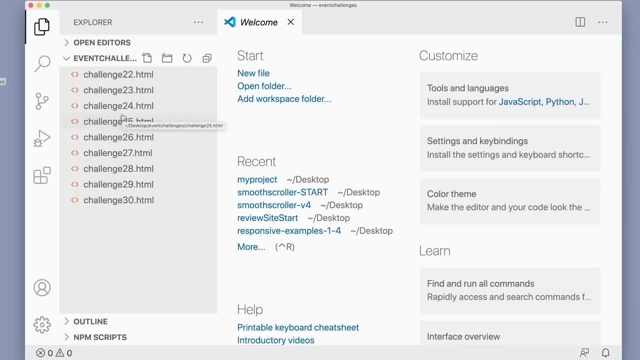 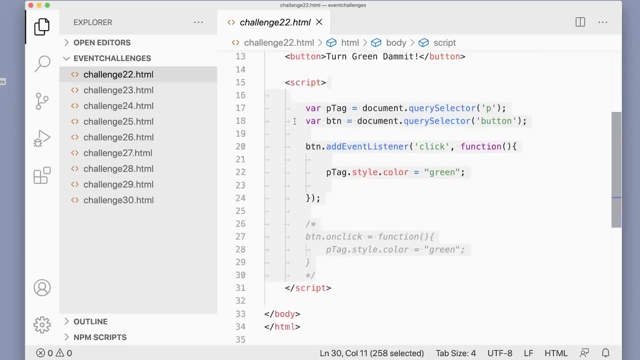 around scope and around some stuff around file management as well and working with scripts and files. So here I have my challenge 22, challenge that I did with the script at the bottom of the page. What I want to do is I want to move the script. 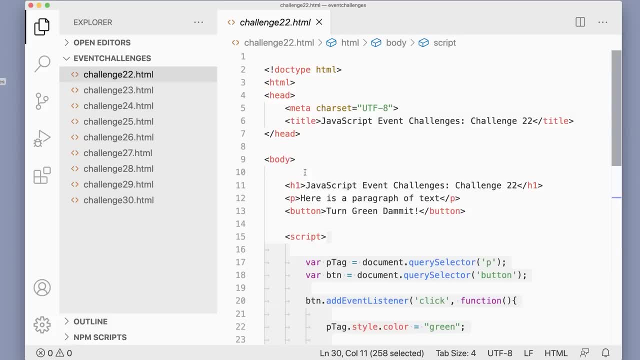 off of the bottom of the page to a separate linked file, and I want to make use of my best practices around the immediately invoked function expression that runs automatically, as well as the use strict directive. that will keep me from accidentally having variables that don't have a keyword. 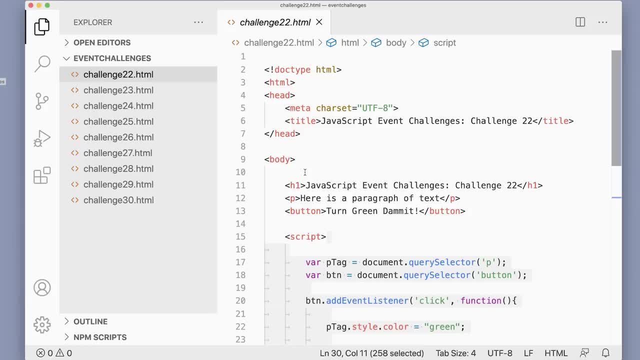 starting them. And then I want to switch my keywords from var to either const or let, wherever I possibly can. So let's do that Over here. I'm going to make a new file and you can click this button here to make a new file. 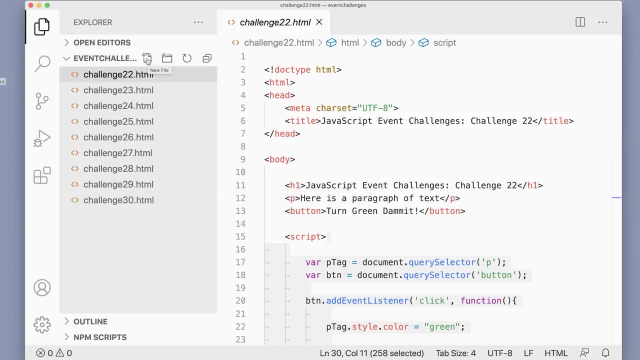 This one makes a new folder, So be aware of the differences there, I'm going to make a new file, I'm going to call it script22.js, to go with this, To go with challenge 22 here And on script22.js. 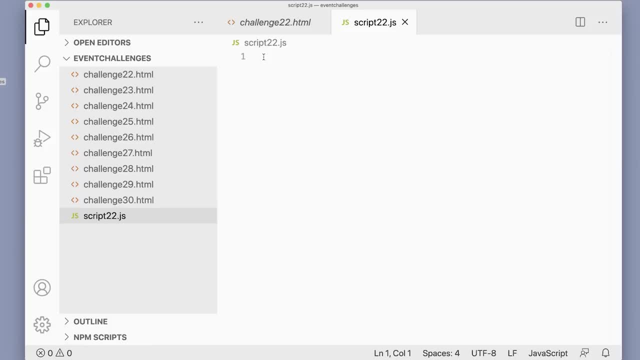 I'm going to start by adding my immediately invoked function expression by starting with the parentheses, and then I'm going to put in here a function with its parentheses and curly braces And then, don't forget, I need one more set of parentheses to make that actually run. 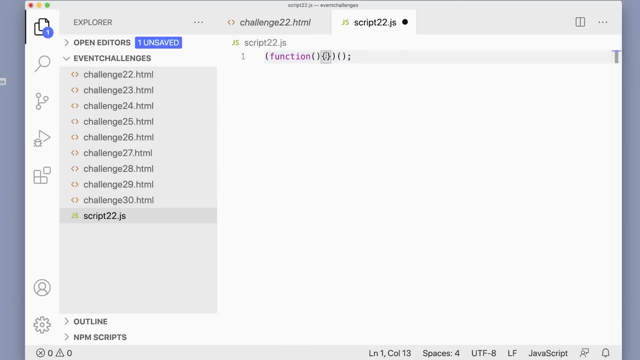 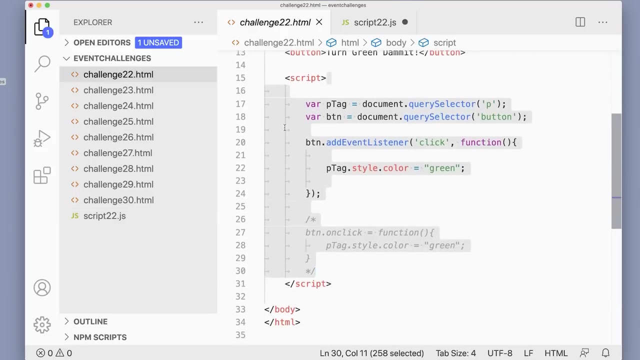 Okay, so I've got a function here And in here I'm going to add the use strict directed. Then what I'm going to do is I'm going to come over to challenge 22 here and I'm going to come down to the bottom. 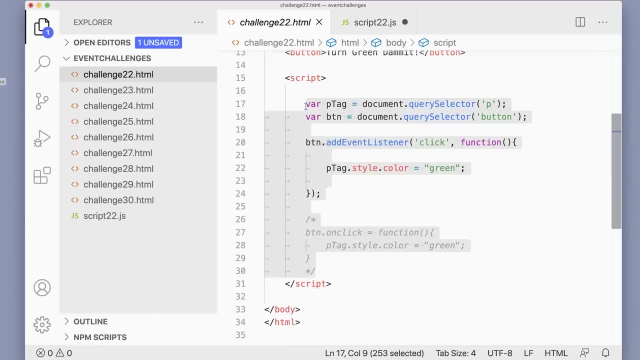 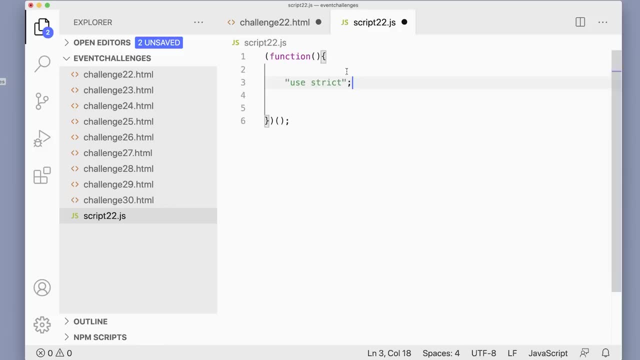 and I'm going to copy or cut. I can actually just cut command X or control X. Cut this script right from here And instead I'm going to paste it in here Like that. Might have to shift tab to move that over. 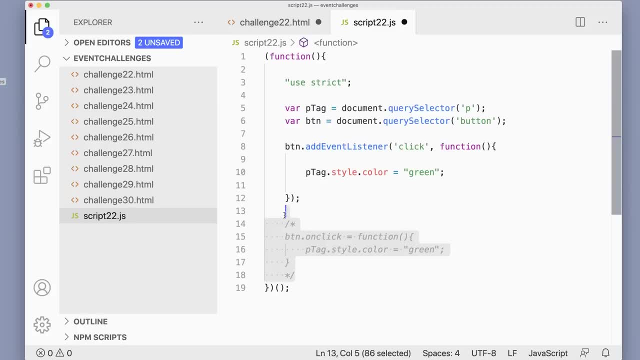 All right, great. So that's here, And maybe I don't need that part so much. That's fine. The next thing I want to do is replace any variable declarations so that they're not using the var keyword. They're using either const or let. 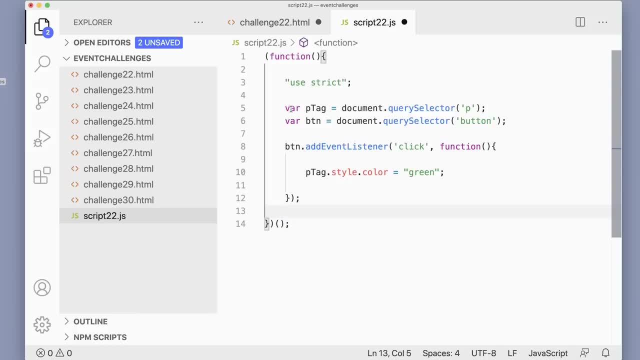 Use const wherever you possibly can And use let where you have to. So this can be const And this can be const. Why? Because I'm going into my document and getting these elements out of the document. That's not going to change. 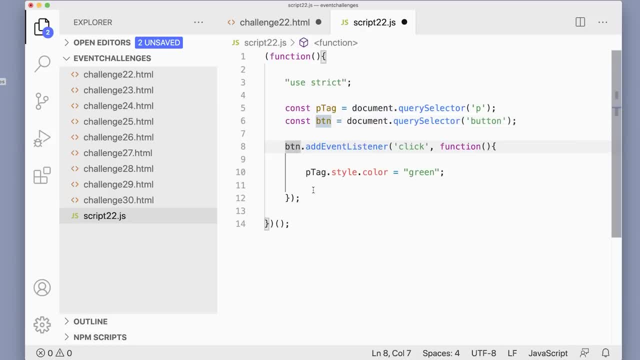 during the running of this script. So that's all fine, That's great. So I've done my three things. I'm using my function expression here, my immediately invoked function expression, as a closure, And then I'm using the use strict directive to 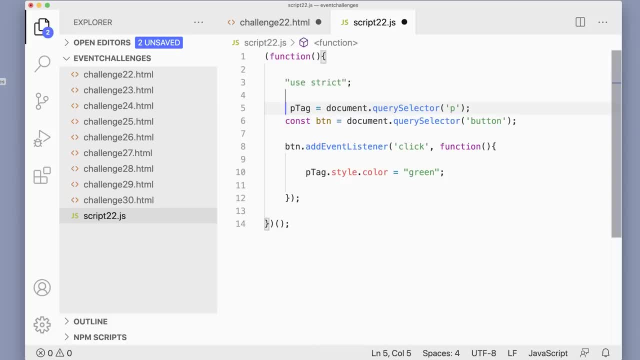 you know, if I had forgotten to put const here, that will catch that problem and tell me explicitly that I've done a bad thing And I've changed my variables declarations from using var to const- Now over here in my file, instead of having the script here. 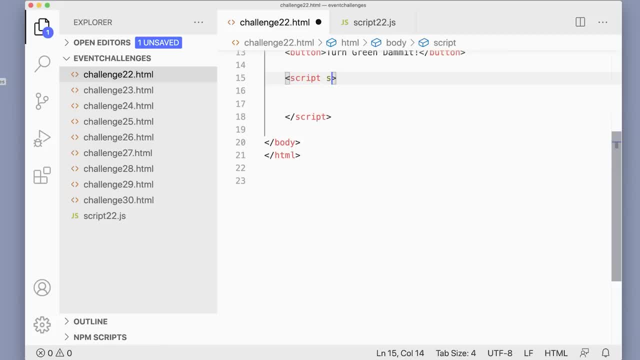 I'm going to do. I'm going to add a source, src equals, And then I can actually put in here script 22.. And that's fine, I can move this up to here, really. So you have to keep the closing tag. 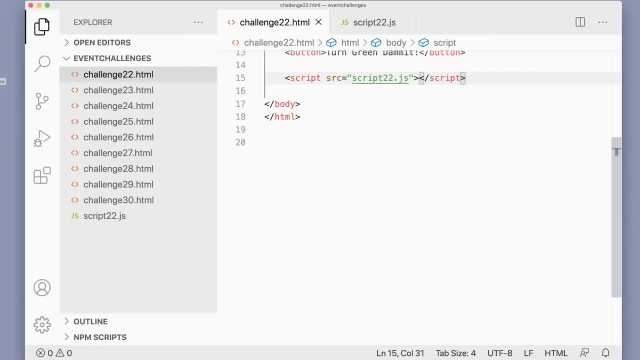 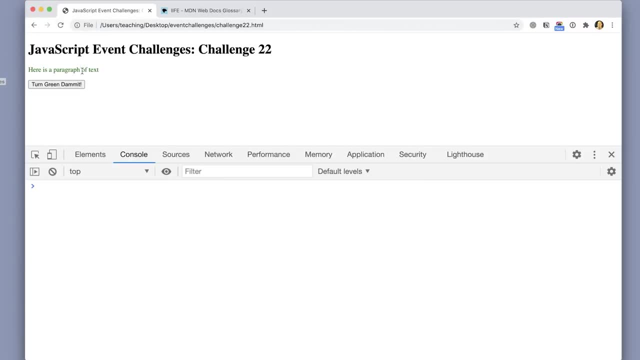 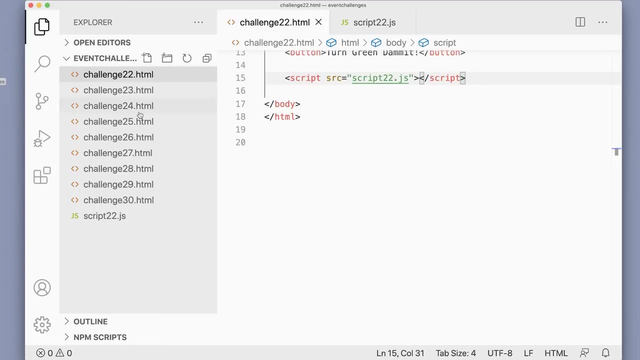 but that will work. And now I can come over to my file in the browser over here. refresh, test it and you can see it still works. It still functions just fine. Even more, if you want to, you could even take this even further. 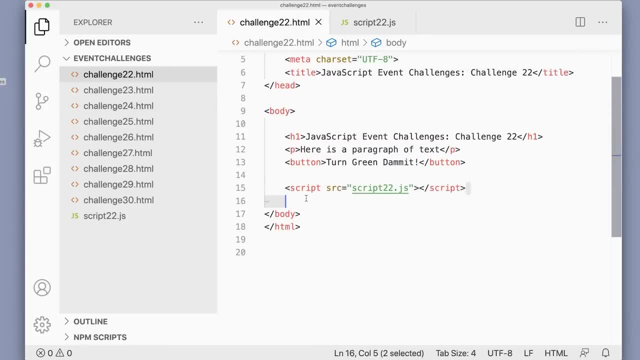 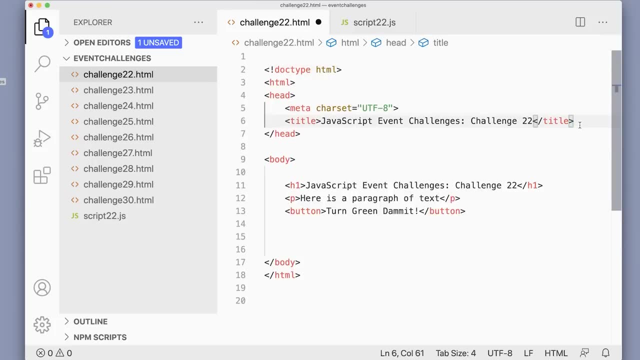 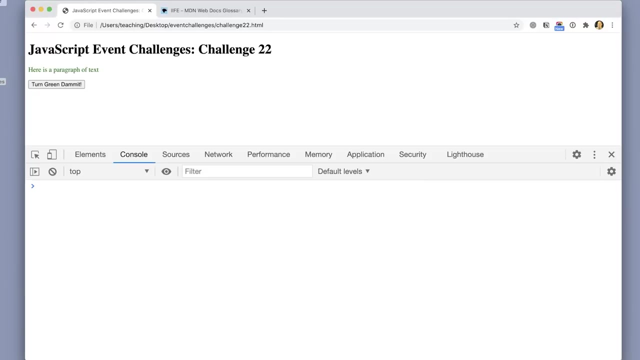 by moving the declaration for the script here up to the top of the file. I can put it in here in the head, but I have to add the defer keyword here With defer. it will make it run as if it's at the bottom of the page. 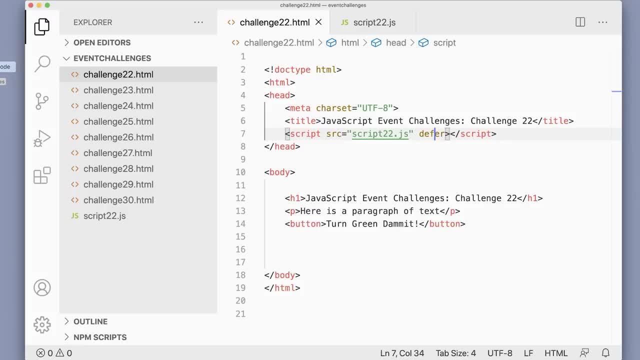 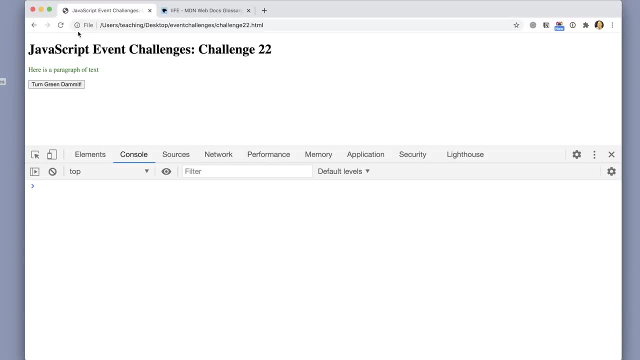 And you'll see that still works If I take defer out of there. watch what happens. Refresh And it doesn't work because add event listener of null. What's going on here is that the page loads from the top to the bottom. 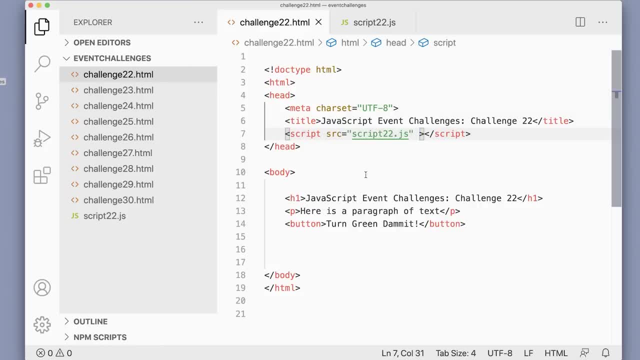 So it's loading the script first before it gets to the button And on the script it's saying: put an event listener on the button. Well, I can't put an event listener on a button that doesn't exist yet, But adding the defer keyword up here. 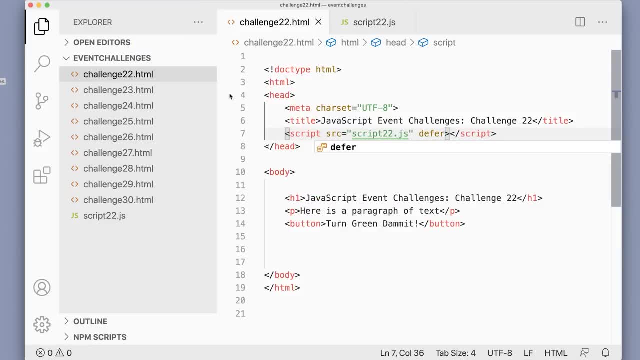 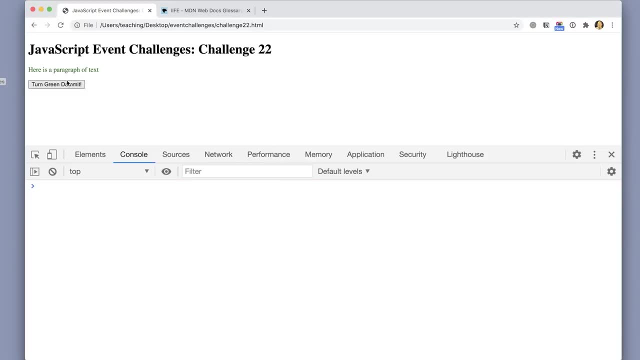 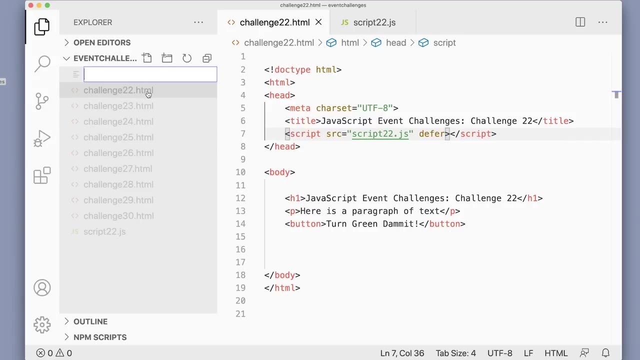 what that does is it makes it so that it loads that script after the rest of the page is loaded. So that will work just fine. So you can go through the rest of these and you'll create a new file for script 23.js. 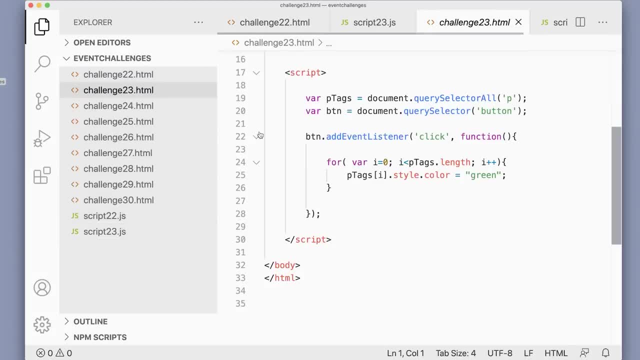 And you'll do the same thing on this one, On challenge 23,. you'll notice that can be const, That can be const. This down here has to be let. That'll have to be let. Go through and put in const and let. 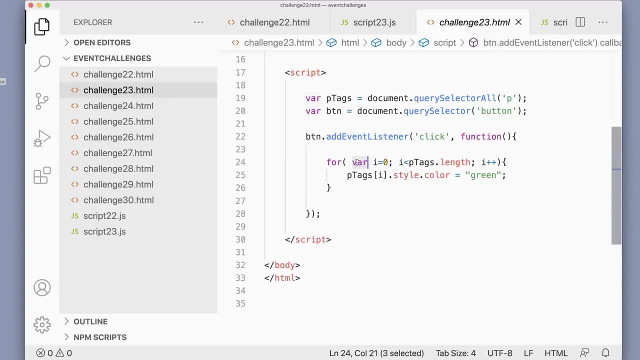 wherever there's a var, Use const as much as you can, And only use let where the variable actually has to change. Here we're using an incrementer that's going to change as we move through this for loop, so it has to be let. 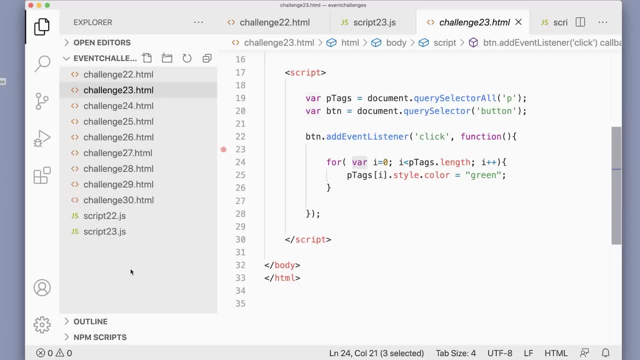 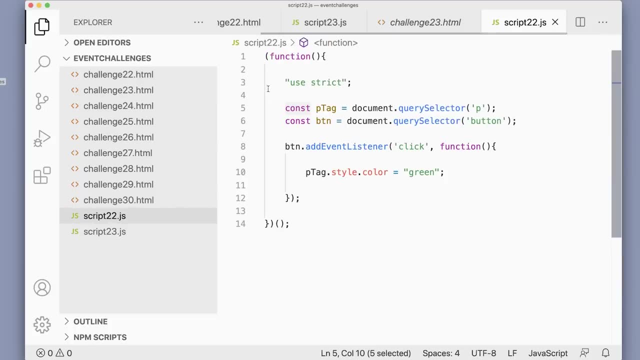 But use const wherever you can, And if you do that and create all these files at repetition you're just eight times. But even just doing that eight times you'll start to really get comfortable with this syntax of the immediately invoked function and using use strict. 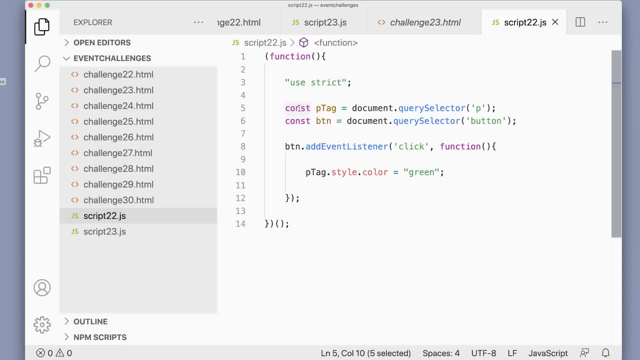 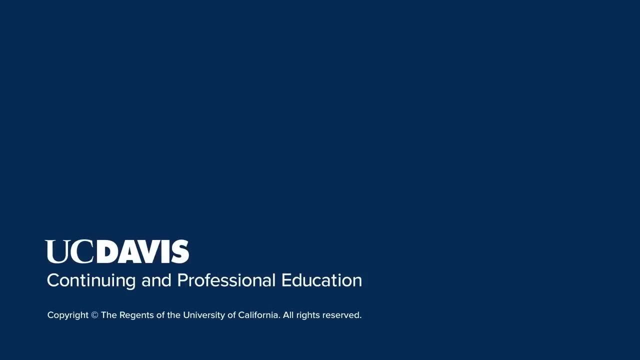 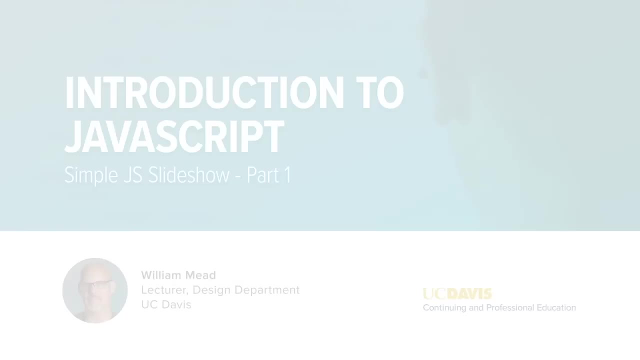 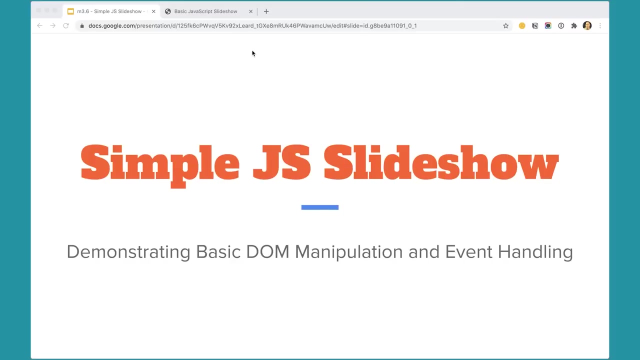 and you'll start to get used to using const and let instead of var for your keywords, And that will really help you out in the long run. Simple JavaScript slideshow Demonstrating basic DOM manipulation and event handling. We've done a lot of the basics. 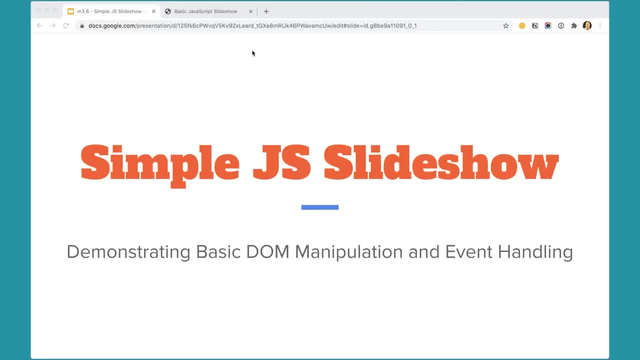 and you've learned a lot about how JavaScript works and how you can manipulate the DOM and capture events. So now it's time to put together some scripts that are actually doing some interesting things and will allow us to test out what we know so far. 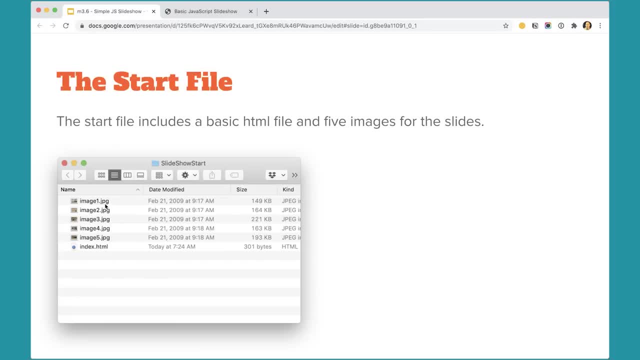 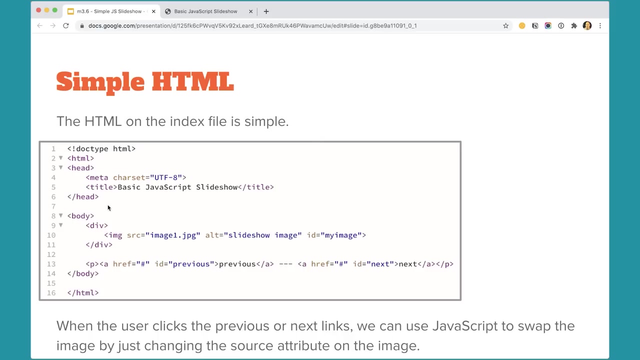 If you look in the start files for this project, you'll notice there are some images and an indexhtml file. If you open up that indexhtml file in your code editor, you'll see that it's just got some very basic markup inside of it. 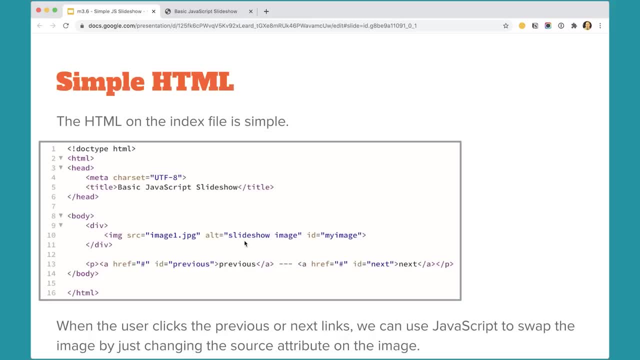 that includes a div with an image- one of the images in the folder- and a paragraph with two links: one for a previous link and one for a next link. If I go to the browser, I can see that it looks like this. 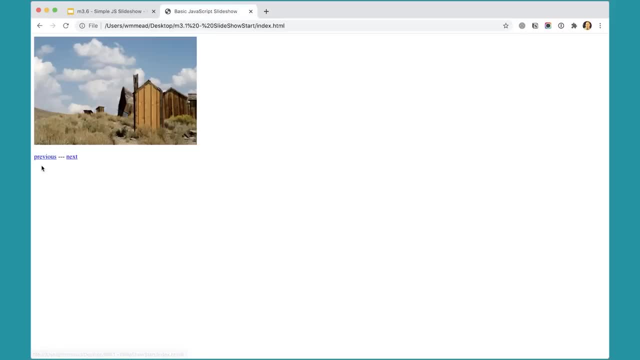 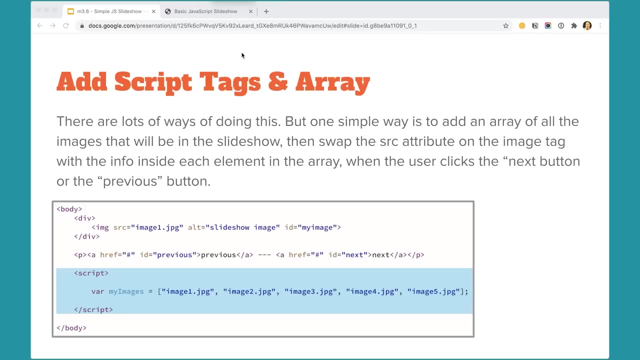 When the user clicks the next link, it'll bring up the next picture, and when they click the previous link, it'll bring up the previous picture, And that's what we're going to make in this particular exercise. here There are lots of ways of going about. 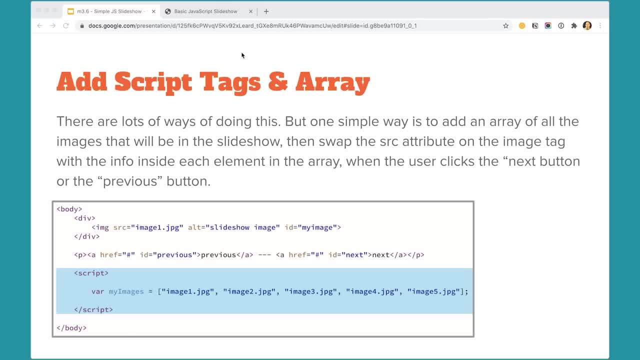 creating this simple slideshow, But one way of doing it is to make a variable that includes an array that includes all of the images that we have in the folder. So let's start right there with that, because that's a really nice simple place to start. 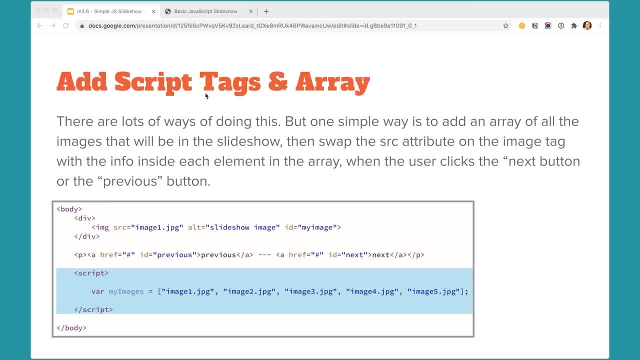 And then what we're going to do is, when the user clicks the link for next or previous, we're going to swap out the source attribute. We're going to swap out the value of the source attribute with the value from this array. So if we're getting 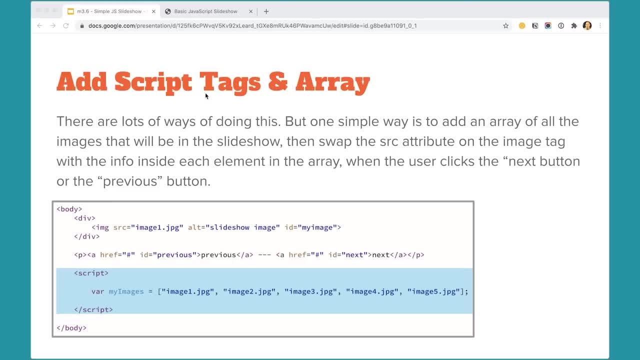 image image. we'll start with getting image zero, which is image one. dot jpeg- number zero in the array And then, when you click next, we'll get image one, which is this one here, which is actually image two. So it's a little bit confusing. 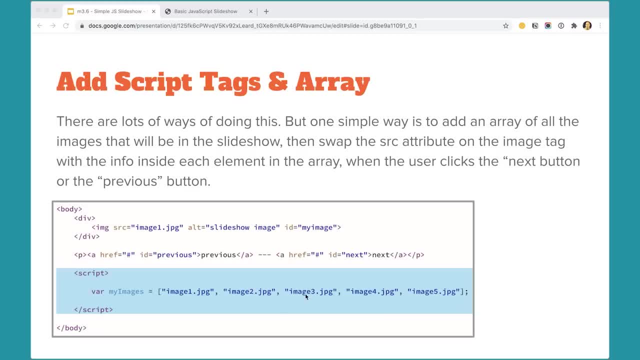 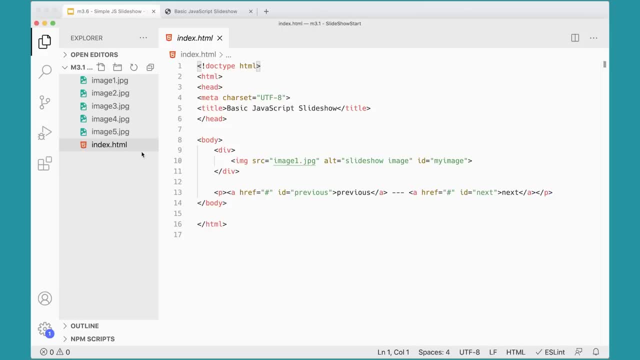 because these are labeled one, two, three, four, five, but they're actually in the array zero, one, two, three and four. But let's start by putting in the array into our script over here, So down here at the bottom of the page. 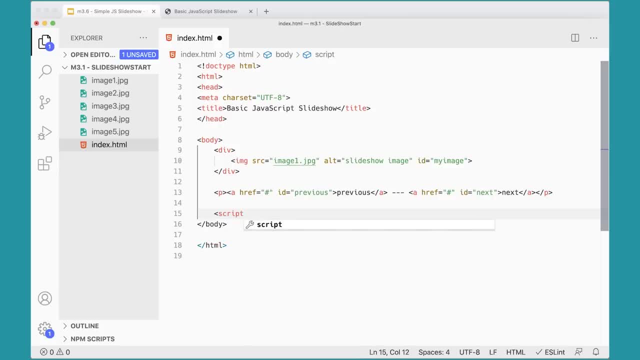 we'll just add script tags like so: Script tags, And in the script tag we're going to add an array var y images equals square brackets, And then each element goes inside quotes. It doesn't matter if they're single quotes or double quotes. 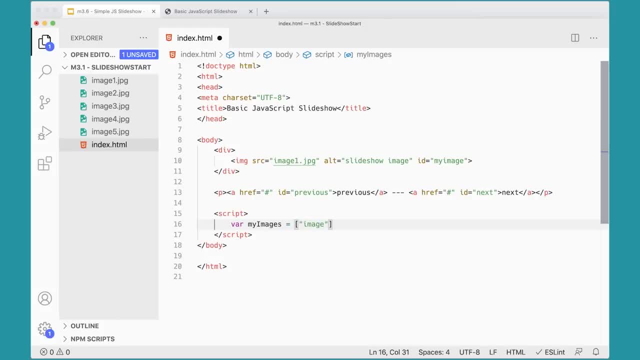 It doesn't really matter, You can do it either way. Image one, dot jpg. comma. image two, dot jpg, and so on. We can actually put a comma here and just copy and paste. That's going to be image three, And then we've got image four. 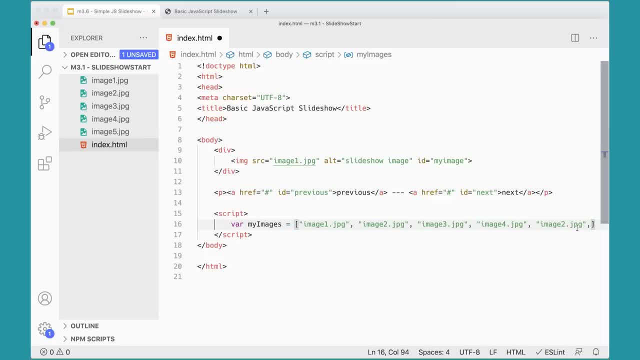 And finally image five, And the last one will not have a comma. It's important you take out that final comma. Image five and then a semicolon. That's our array. So there's our array And that's going to go and get these images. 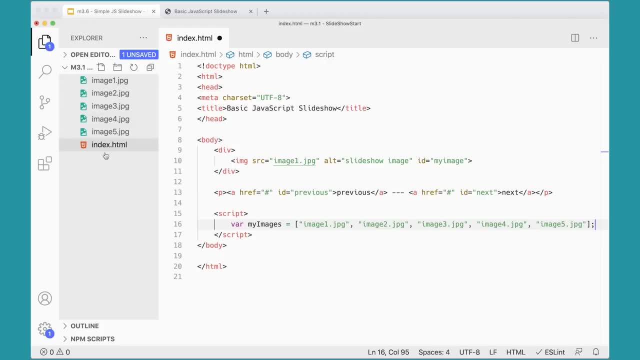 And they're all in here in the folder. If we had a folder over here called images, you would just add that here. You could add images slash and add the folder name in there. But we actually in this case with the files I gave you. 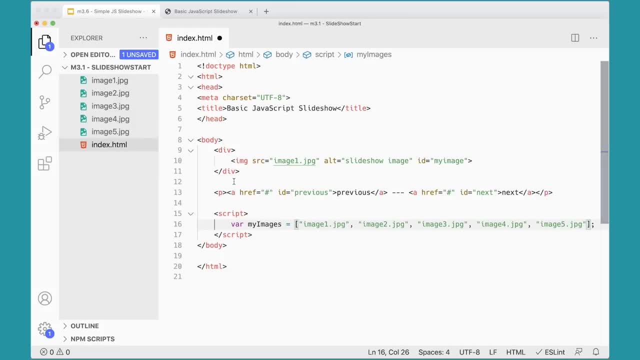 I didn't create a folder for them, So they're just sitting here kind of at the root level of this folder. So that's great. So that's our array of images. that describes all of the images that we have here, And next we'll start working on. 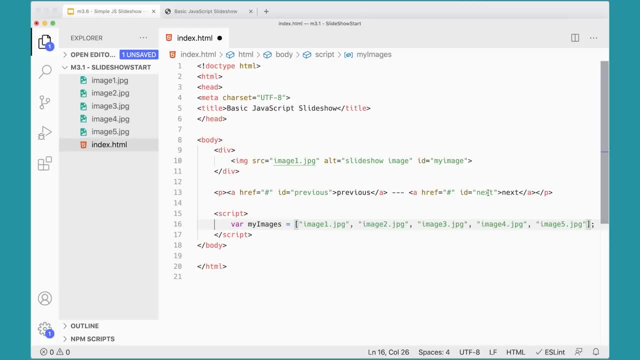 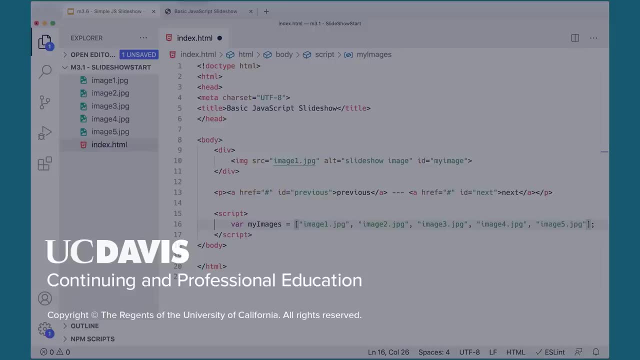 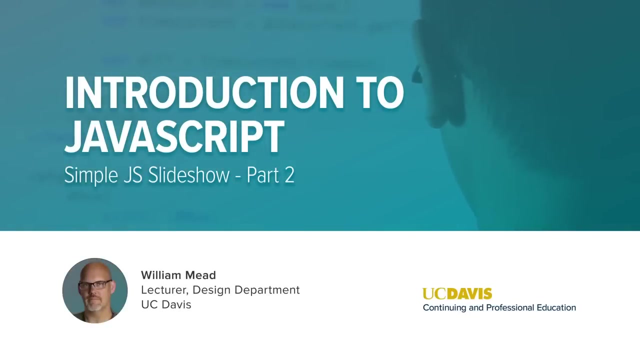 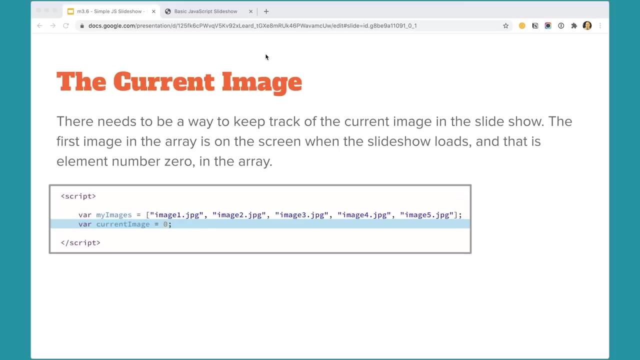 how to actually capture the event of clicking the next button and then handling the swapping of the source attribute. You will need some sort of variable that we've discussed along the way to capture which image that we're actually on in this array. So I'm going to make a variable. 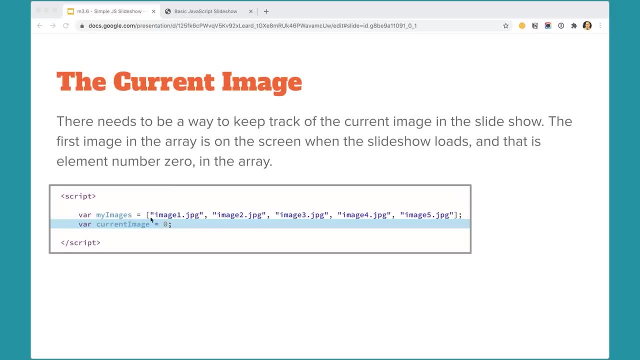 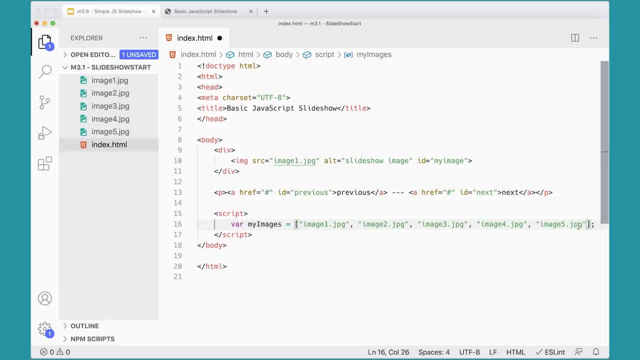 called currentImage and I'm going to set it to zero because when the page loads, this image is showing, which is number zero in the array. So images square bracket zero would get that image. So let's set that over here, Let's make a variable here. 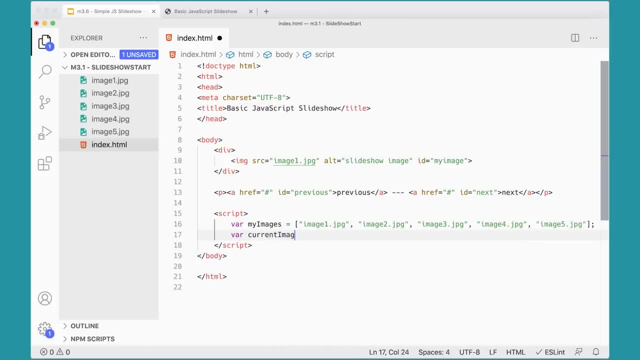 barCurrentImage and set that to a value of zero to start with. So there we go. So that will help us with that, And then from there we need to create an event handler that will handle the clicking for the next button. We'll do the next link first. 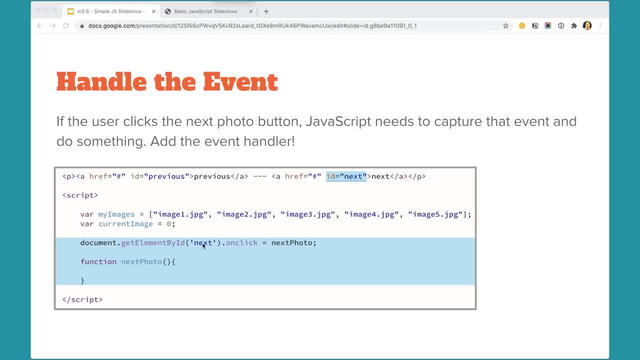 This is what it will look like: Document getElementById next. So it's going to go into our document and find that link that has the ID set to next And I'm using the onClick specialEvent property And I'm going to run a function. 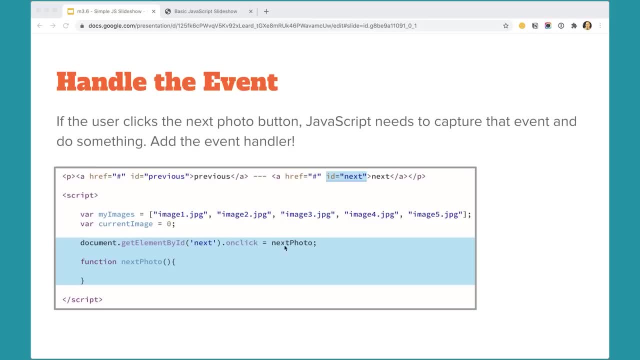 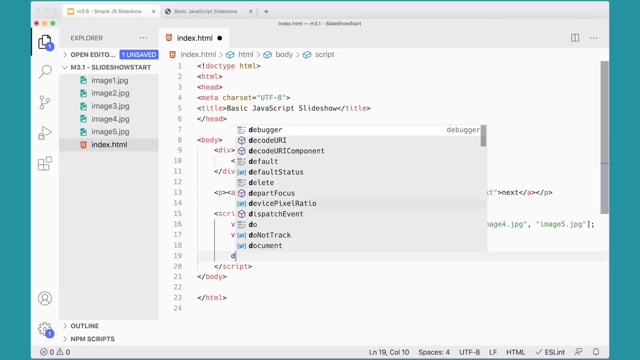 called nextPhoto. Notice: it doesn't have parentheses at the end of it, But I'm going to assign it a function called nextPhoto, so then I can create that function, nextPhoto. So let's go ahead and add this to our script Document. 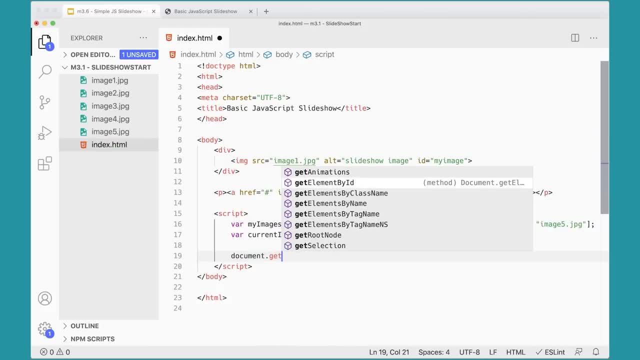 getElementById. Make sure it's always a good idea to pick it from the list so you don't spell it wrong. You have to get the capitalization right Next. So that's going to go in here and look for this link here that has the ID of next. It's going to go into our document. 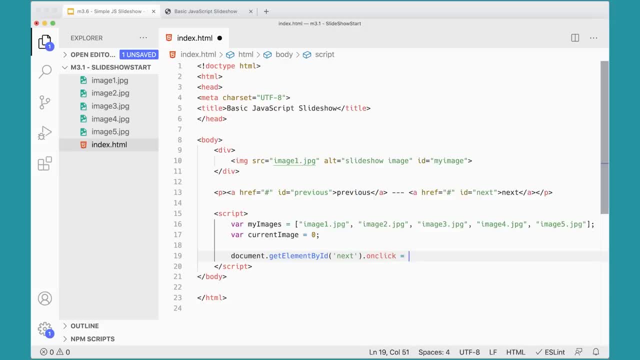 and look for that. onClick equals nextPhoto semicolon, And then down here we're going to make a function called nextPhoto like. so There we go. Notice that if we look at this image tag here, it has an ID called that has a value set to. 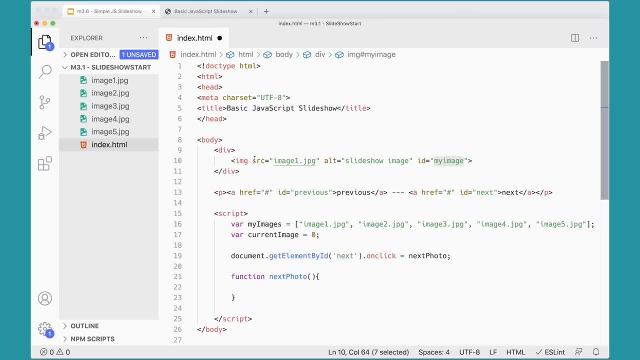 myImage. So that's what we want to get, And we want to change the source attribute on that image if this button has been clicked. Also, what we want to do is we want to take currentImage here and increment it. So I'm going to do that. first, I'm going to say: 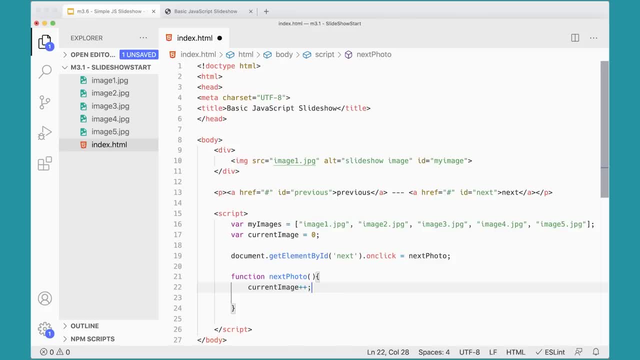 currentImage plus plus. And remember that's the same as saying: currentImage equals currentImage plus one. Doing currentImage plus plus is just a shortcut For taking currentImage, adding one to it and assigning it back CurrentImage plus plus. So that's just a shortcut. 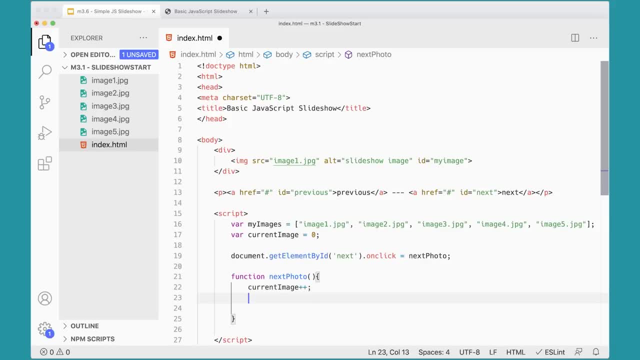 Okay, great. So now I'm going to say I'm going to come in here and I'm going to say I need to go document dot, getElement by ID. What ID do I want? I want myImage up here, myImage, And I want to set. 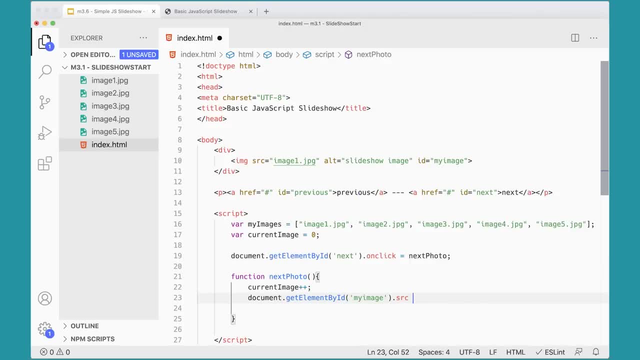 its dot source src equal to myImages. that array currentImage. So that will go into this array here and find currentImage. Now, the first time I click that link, currentImage is going to get incremented to one, So it will come in here. That's zero. 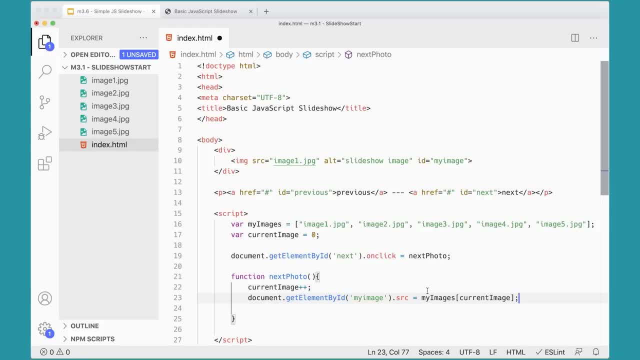 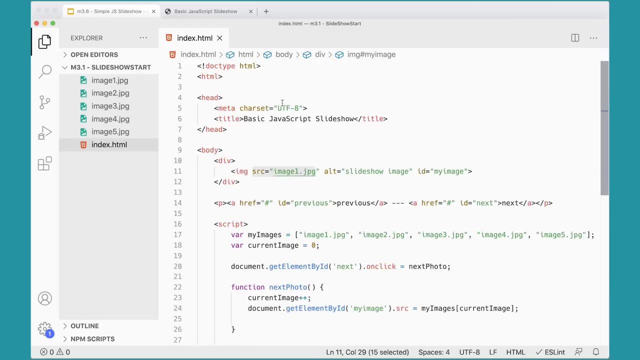 So it says: okay, that's image2.jpg. So this is going to be image2.jpg and I'm assigning that to this src attribute up here, This src. So instead of saying image1.jpg, it's going to say image2.jpg. Let's save that and see. 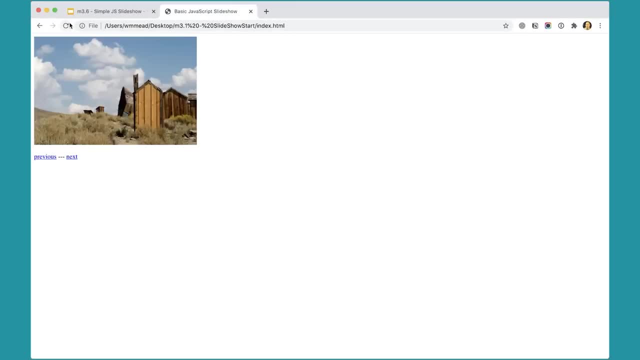 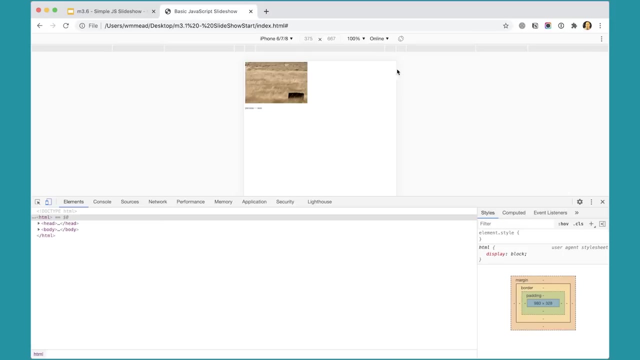 if that works, Come over here refresh. If I click next, you can see that it's changed. And if I do inspect down here, let me arrange this the way I want it. I'm going to put this down at the bottom. I'm going to turn off. 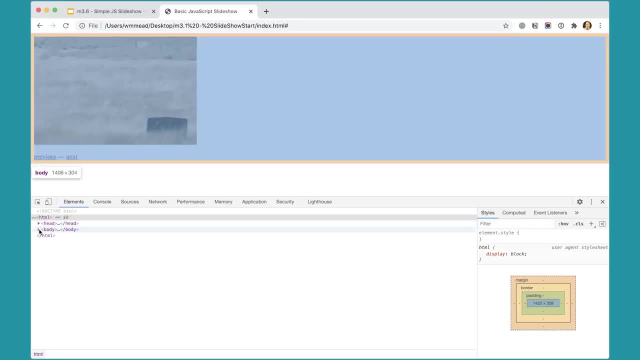 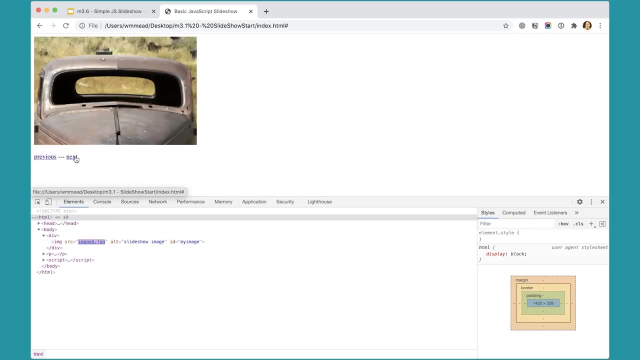 that button there. but if I come in here and look at this div, notice the src says image2.jpg. If I click next again, notice that got changed to image3, image4, image5. Oops, What happened? We got to image5 because there are five images. 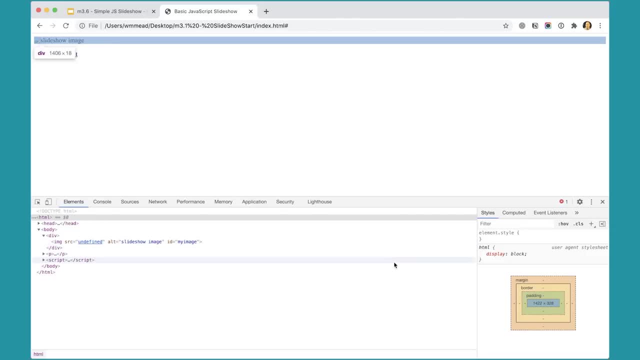 and then I clicked next again and now I have undefined and you'll notice there's an error over here as well. so I can go to my console log and see undefined error file not found. so it could not find I've gotten beyond the end of my array. 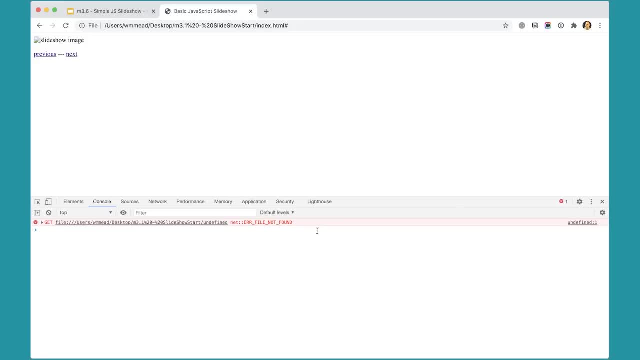 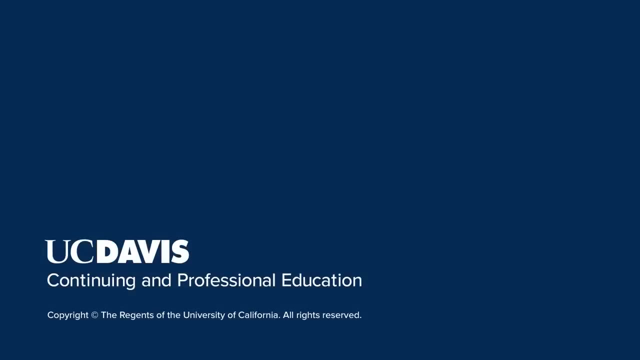 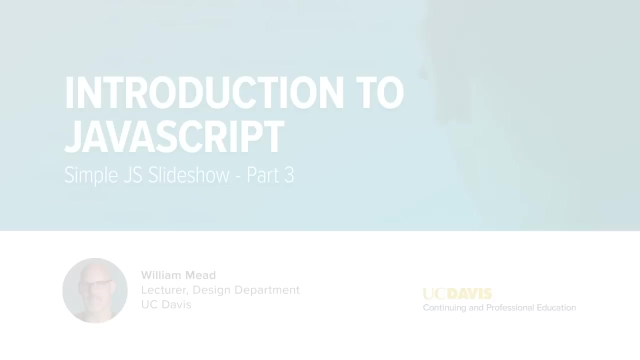 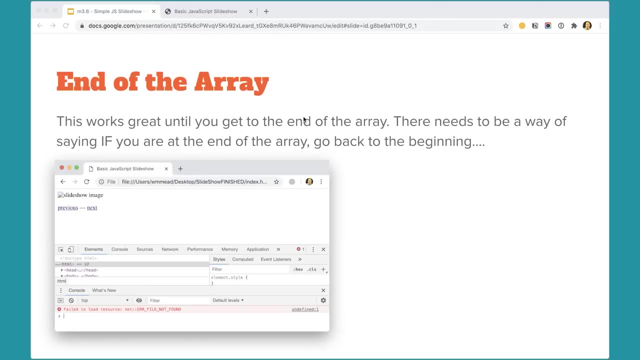 so at a certain point it ceases to work, depending on how many pictures are in the array. so that's what we're going to fix next. Let's think about this for a minute. What we want to do is we need some code that says: if you're at the end. 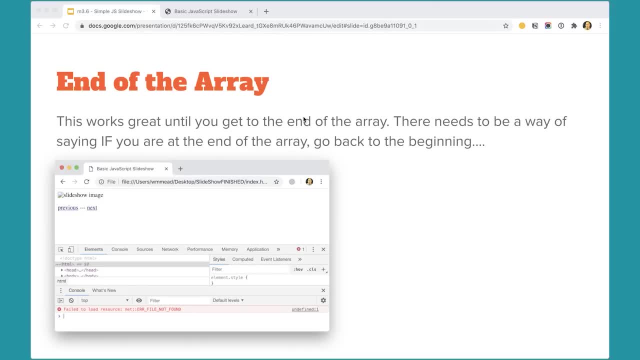 of the array. go back to the beginning. Think about that for a minute. What do we know about JavaScript that will allow us to do this kind of thing? What logical flow control structure can we use to handle this? If you were thinking of something like this: 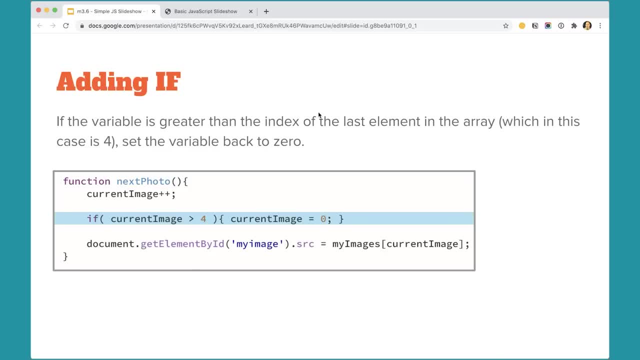 you're on the right track. So, if currentImage is greater than 4, because, remember, the numbers in the array are 0,, 1,, 2,, 3 and 4, so if it gets greater than 4, if it becomes greater than 4, 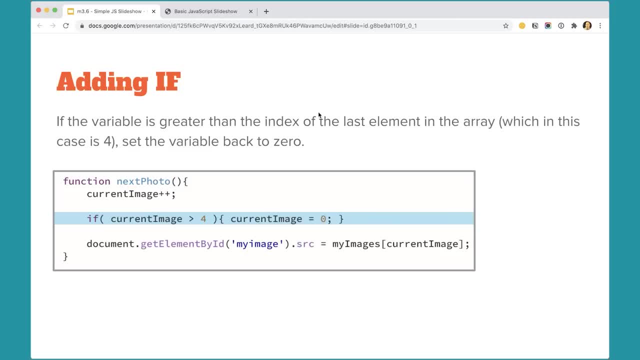 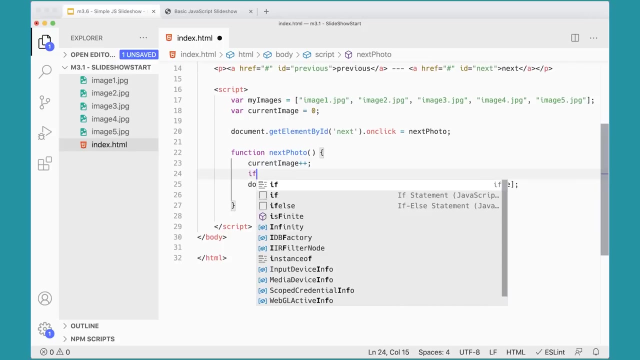 we can set currentImage back to 0 and then go ahead and get the next image. So with this if statement in place, you can make the slideshow effectively loop around. So let's go ahead and add this, And it's just going to go in here. if 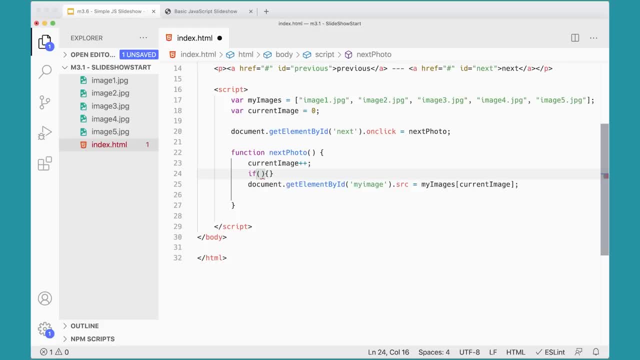 parentheses: curly braces. So in the parentheses we want to say: if currentImage is greater than 4- And it's kind of nice if you put some extra spaces in here, although not really necessary- If it's greater than 4, then the value of currentImage is going to get set back to 0. 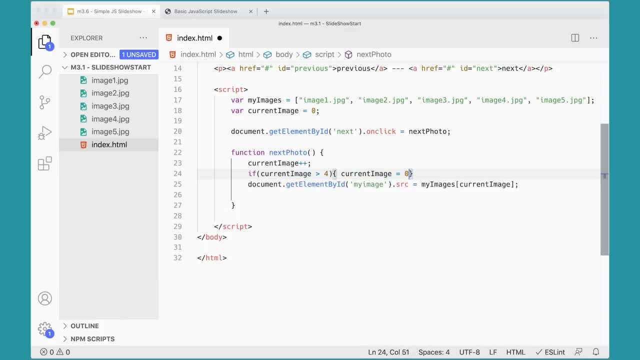 currentImage equals 0 And we can just do this on one line. sometimes you're likely to see it more like this, like that perhaps, but this is such a short one statement, selection, if statement, that it kind of makes sense to just keep it on one line there. 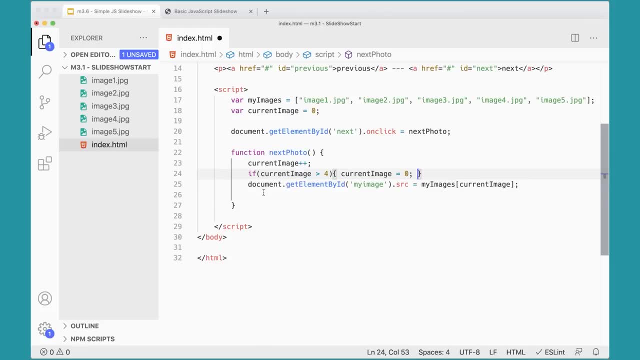 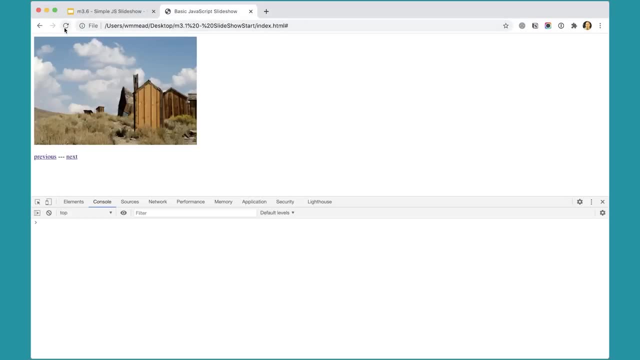 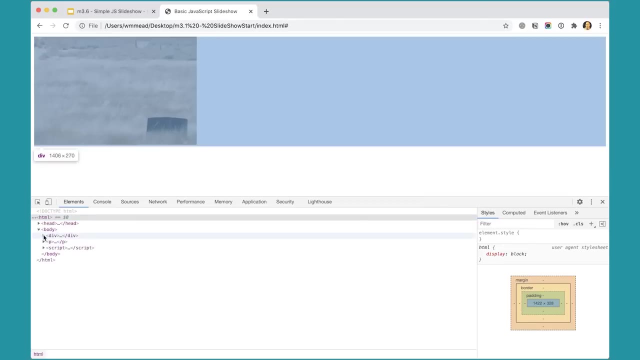 If currentImage is greater than 4, we can set that back to 0. Let's test that. I come over here and refresh this and I click next and down here in the elements I'm going to come down and see in my div you can see that's image 2. 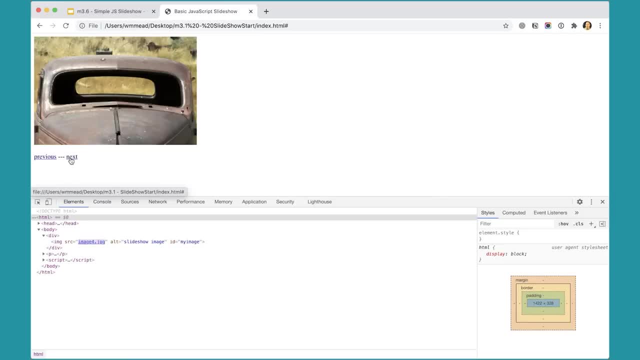 next 3, next 4, 5 and then, if I click next again, it should get set back to 0, which would get us image 1, and that works. So now the next button is looping around through all of the images that we have. That's great. 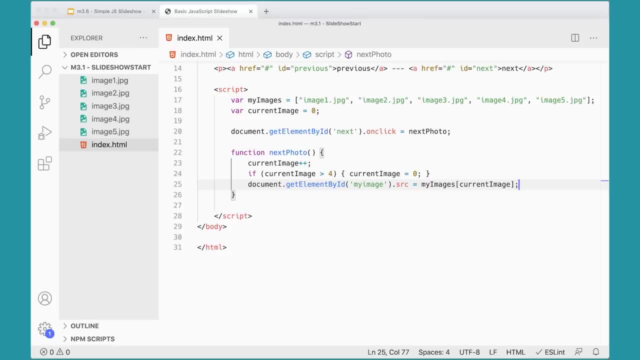 Now it would be a little bit better if we could generalize our script a little bit, So, rather than greater than 4 here I know that it's 4 because I know it's 0,, 1, 2,, 3, and 4- 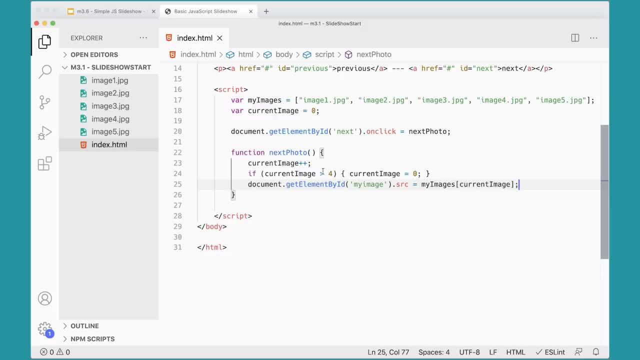 I can use my length property to get that I could do is less than myImageslength. That's not quite right yet, because the length is 5, 0, 1, 2, 3, 4, 5. There's 5. 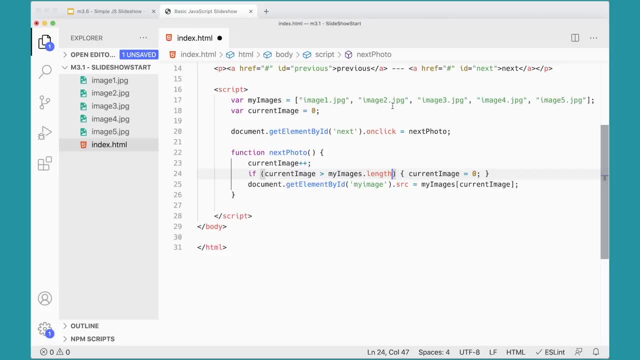 1,, 2,, 3,, 4, 5. There's 5 images in here. That's the length, But the images are numbered 0,, 1,, 2,, 3,, 4 And we know that we want it to be 4. 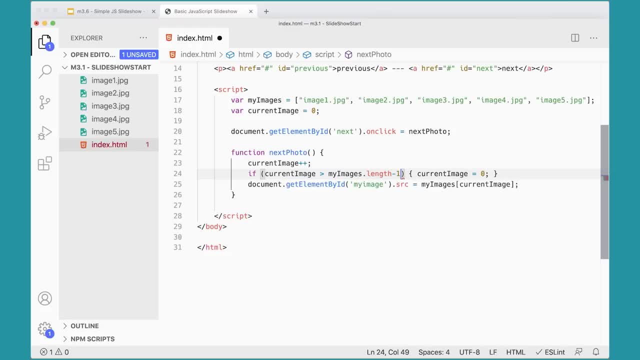 So it's myImageslength minus 1, And that may feel a little strange at first, but we'll be using this a lot when we're working with arrays. The length of the array minus 1 is often what we want, because arrays start counting at 0. 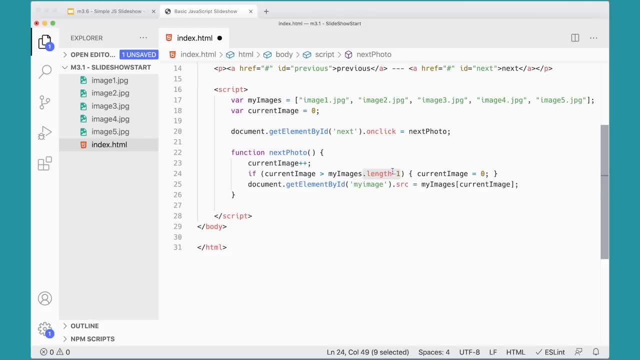 0,, 1,, 2,, 3, and 4. So myImageslength minus 1 will give us a 4, And it's generalized so that if I were to add more pictures in here and add more pictures into the array, then the script would continue to function. 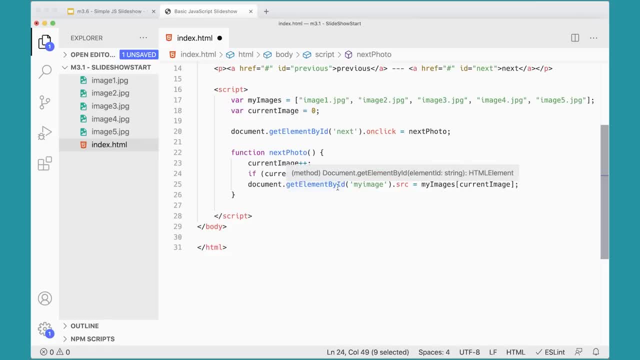 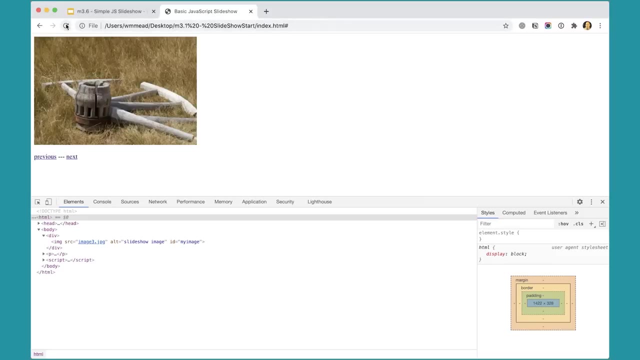 without having to go in and adjust the script as well, And wherever in programming we can do that to make it so that there are fewer adjustments in the future. if you change things, the better. That will make your script more general. So let's just test this just to be sure it still works. 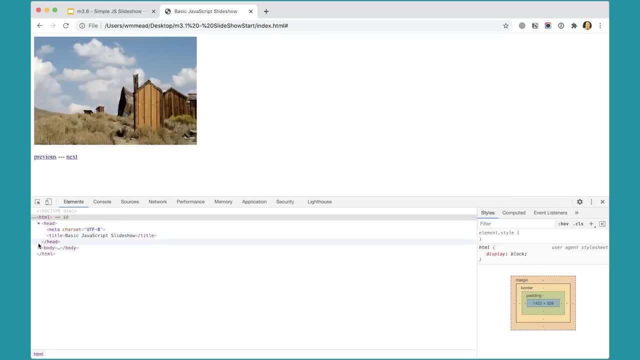 And, sure enough, the page loads and we've got in our body, here in our div. we've got image 1 here and I can click next, I can click next all the way through and it'll wrap around to the first one just fine. So that's great. 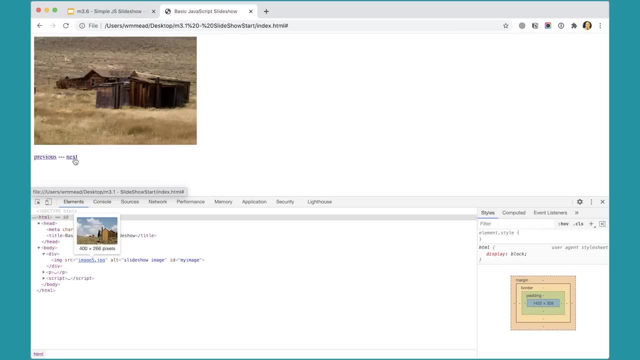 Okay, Next thing we need to do is handle the previous button, And maybe you can do that for yourself. It's always a great challenge. It's not that different than what we just did. It's a little bit different, but it's not that different, So you might be able to do the previous button by yourself. 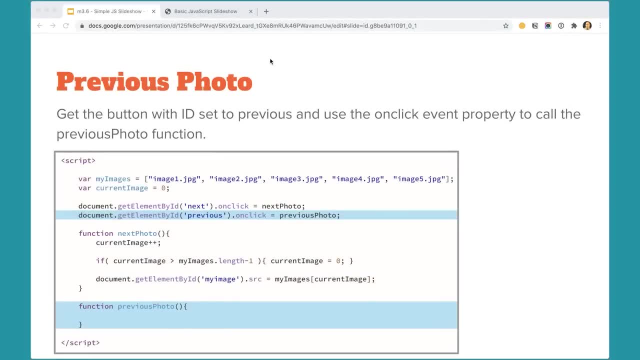 To get started with the button for getting the previous photo, we first need a event handler that will go in and find that element with the idea of previous and add the onClick event property and run a function called previousPhoto, and then we can set up that function. 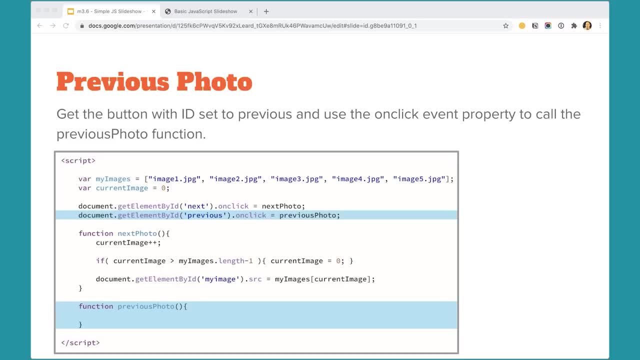 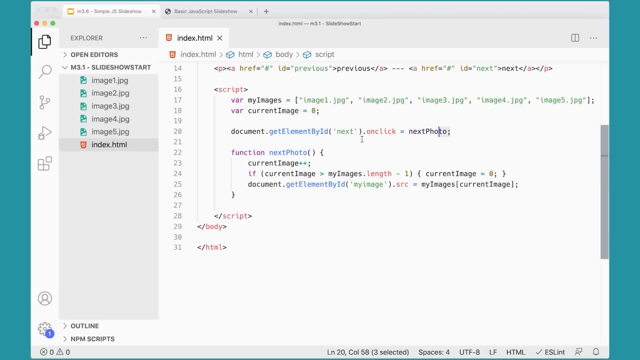 So let's do that first. So up here- and you could even copy and paste this if you wanted to. Sometimes it's best to do that just to avoid making mistakes, but you have to be sure to change everything you need to change. So, instead of next, this is previous. 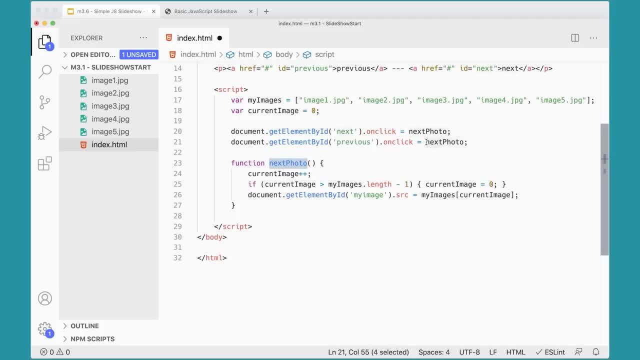 instead of nextPhoto is going to be previousPhoto. Okay, So now we've got our event handler and now we need a function again. copy and paste, always good to make sure the names match function. previousPhoto. parentheses, curly braces. there we go Now the way to think about this. 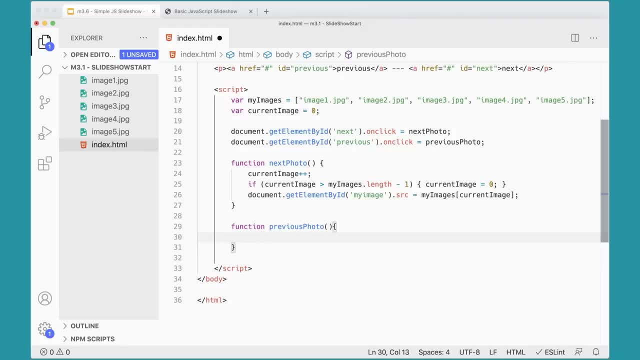 the previousPhoto button. you have to think backwards and the easiest way to do it is to think about what happens if you're on the last photo. suppose we're showing on the screen image 5 and currentImage is currently set to 4. what do we want to have happen? 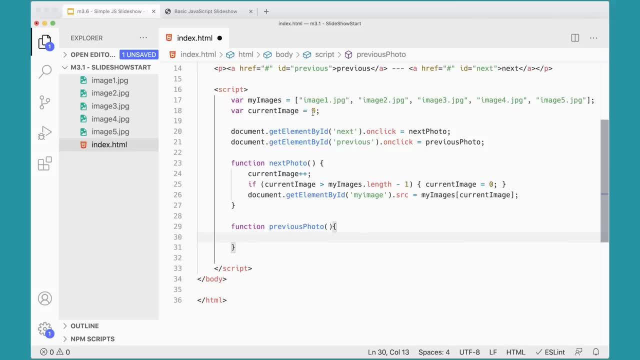 when we click the button previousPhoto, we want currentImage to decrement, we want it to go from 4 to 3, and then we want to go in and get this image and then, when we click it again, it goes from 3 to 2 and we get that image. 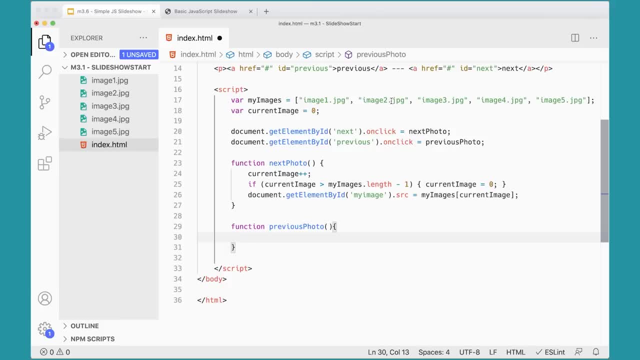 and then it goes from 2 to 1 and we get that image. and then it goes from 1 to 0 and we get that image. if you click it again, we don't do some sort of if statement- it's going to go from 0 to. 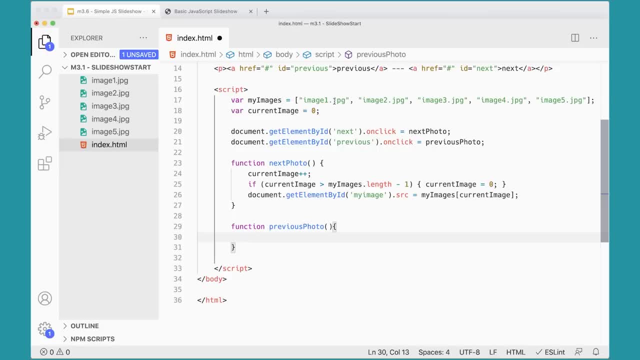 minus 1, and that's not going to work. so if the, if the value of currentImage is less than 0, if it's less than 0, we want to set it to. what well, we could set it to 4, that would work, or we could set it to. 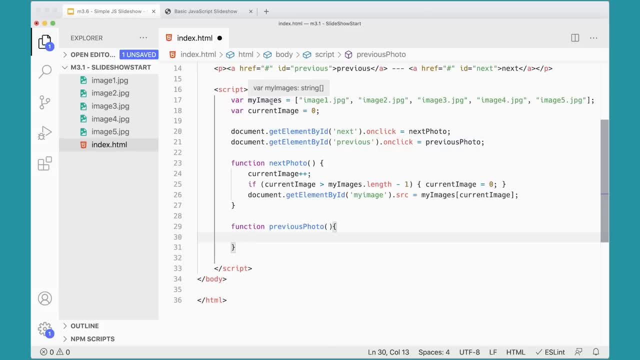 myImageslength. myImageslength minus 1. right, let's take this piece by piece. let's do this part first. I'm going to decrement currentImage. current image, oops, minus, minus. that will decrement it. that's the same as saying currentImage equals currentImage minus 1. 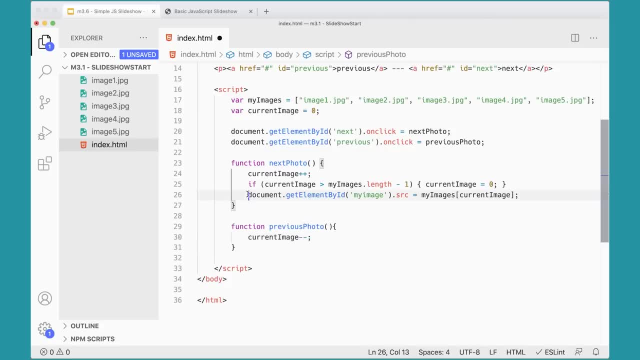 so we're going to decrement currentImage and then we can do this again if we leave off the if statement altogether. you'll see when we get down to the bottom of the images we're going to have an error. but let's just do it, just to see how that happens. 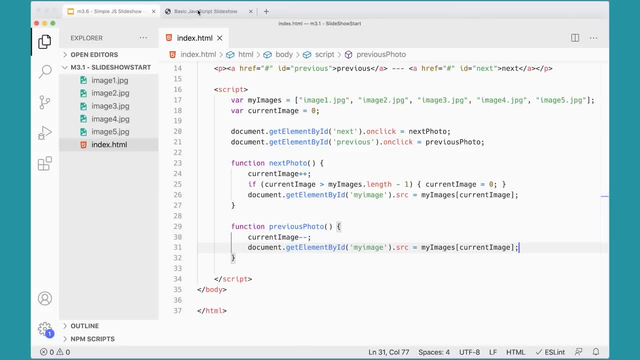 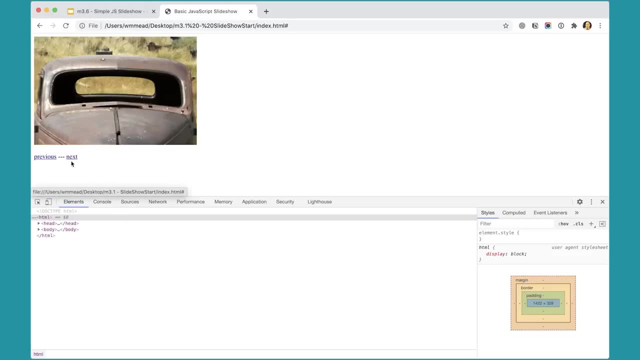 and what that looks like. so over here I can refresh this and I'm going to click next until I get to the end, to the fifth photo here. oops, I'm going to click next. so I'm on 4. one more, so now I'm on 5. 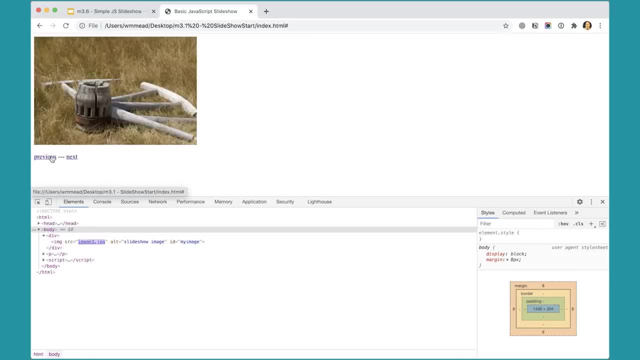 and now I can click previous and it'll go to 4, it'll go to 3, it'll go to 2, it'll go to 1 and now, if I click it again, it's going to have an error, because currentImage is going to be minus 1. 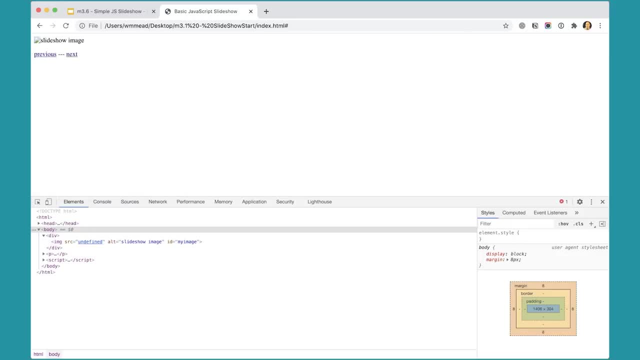 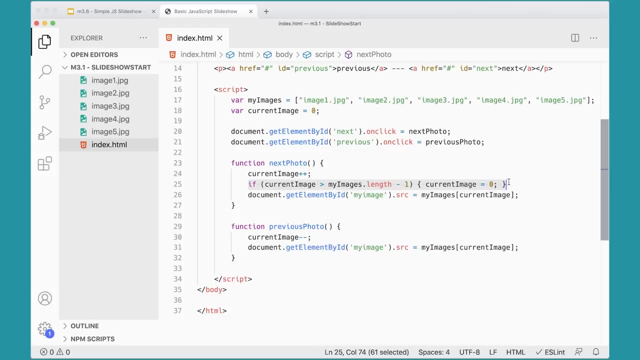 and that's not going to work. okay, undefined. so that's where we need our if statement. so let's come back here and see if we can write that if statement. so I might as well copy this one and paste it in here, but instead of. currentImage is greater than my images. 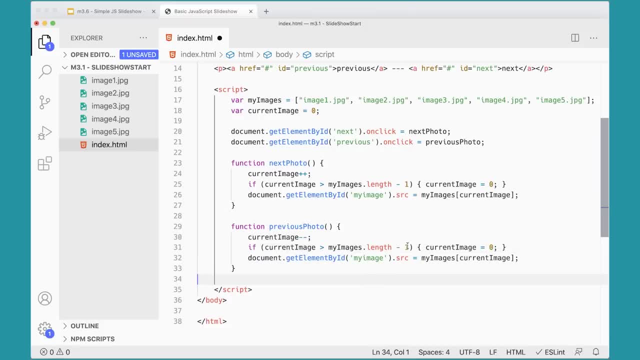 what I'm really looking for is: is currentImage less than? is it less than 0? is currentImage less than 0? and if it is, I could set currentImage to 4 and that would work, because that puts it back at the end of the array. 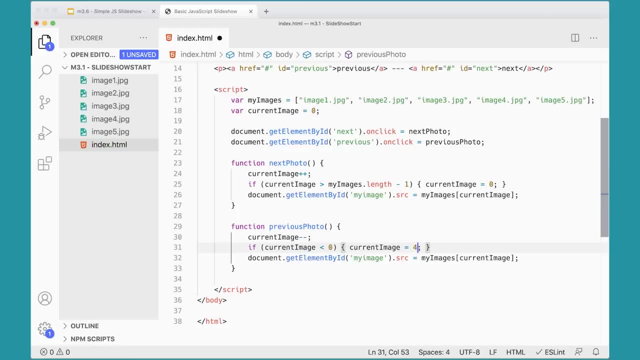 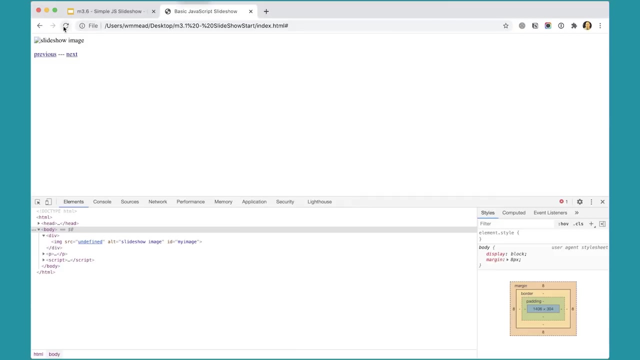 that'll work just fine. but even better is to use the myImageslength minus 1 again to keep the script generalized: myImageslength minus 1. so now you'll see. if I do this, I'm going to come back here, refresh the page and again I'll go back up to the end of. 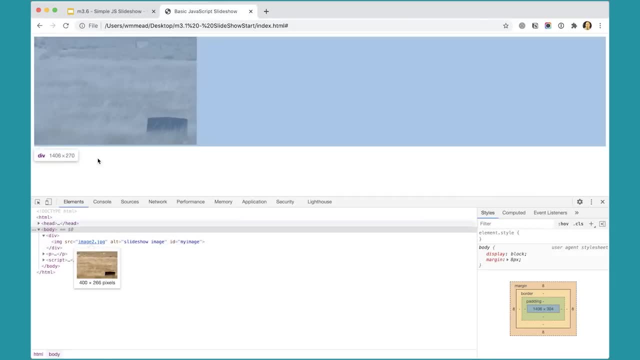 the list here there's 2, 3, 4, 5. ok, now, if I click previous, it should go to 4, and then to 3, and then to 2, and then to 1, and now, if I click it again, currentImage is now going to be minus 1. 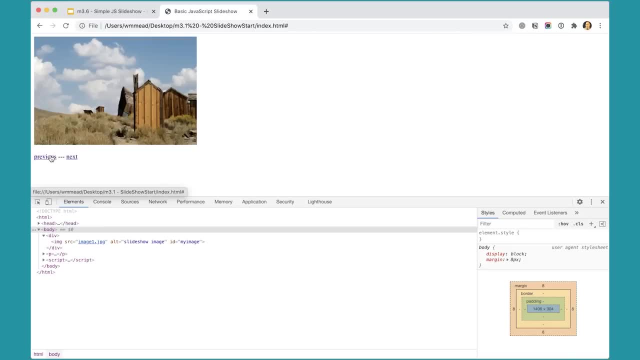 that's less than 0. that's going to kick off that if statement and say, alright, it's less than 0, that's less than 0, and there it is. there's 5 again because currentImage is 4, which is getting image 5 from the array. 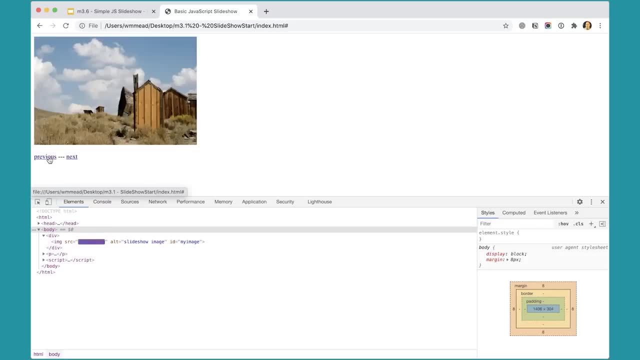 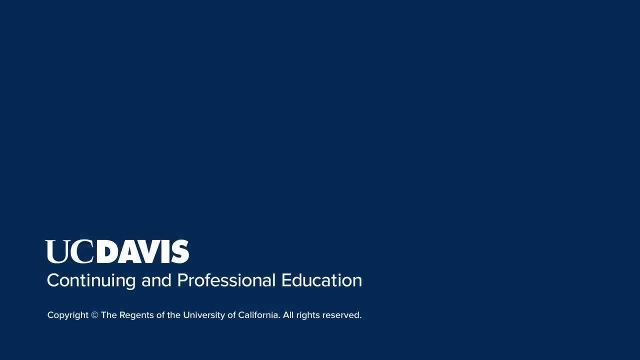 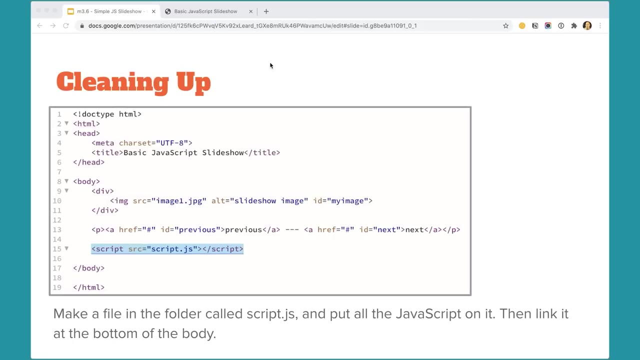 so now I can loop through in either direction. I can loop through going frontwards and I can loop through going backwards. everything is working. now all we need to do is clean up the script just a little bit, make it a little bit better, and one way of doing that is to put it in a separate script file. 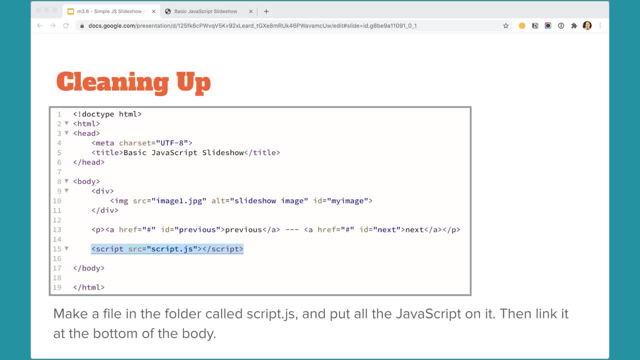 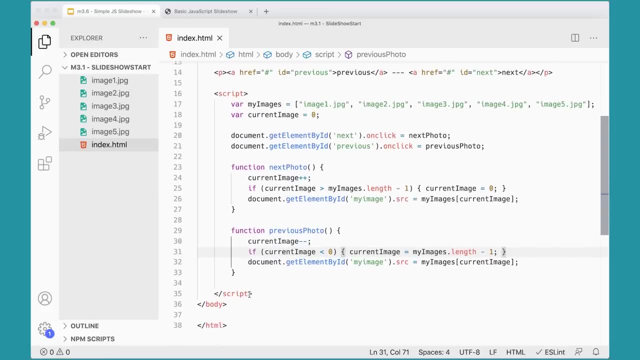 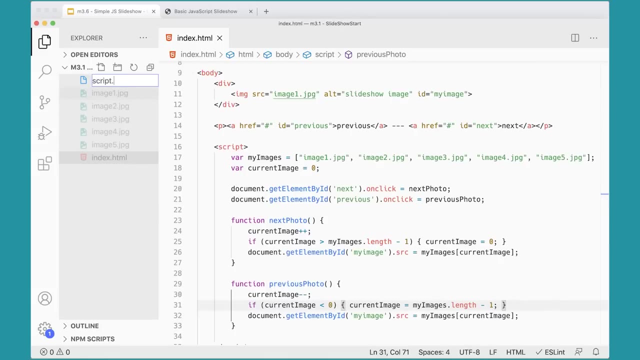 for this script. it's short enough. you could leave it at the bottom of the page if you wanted to. but just to practice our best practices, let's move this script into a linked file, so over here I could make a new file and call it scriptjs. 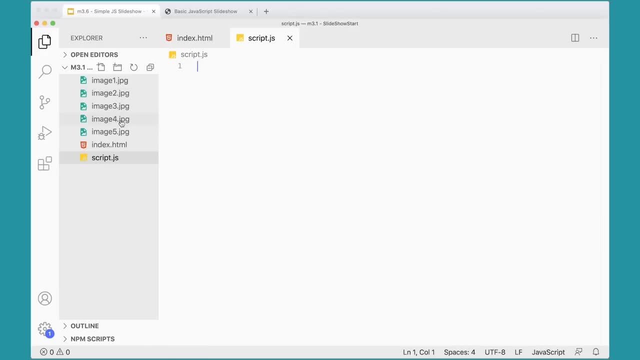 and on this file I could put my, my, my, my, function expression that will be immediately invoked. so we do that with parentheses and then in the parentheses we put in function with its parentheses and its curly braces, and then one more set of parentheses and a semicolon. 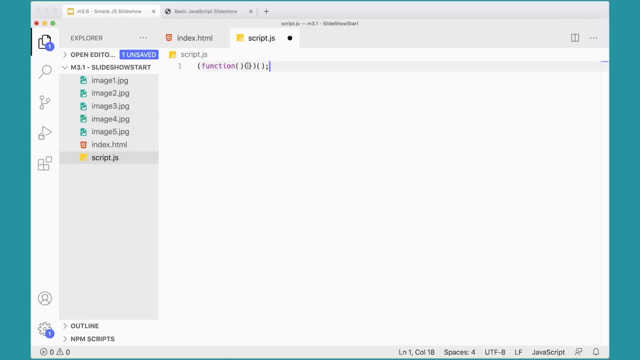 terrible syntax, but this will run when the script runs, when the script loads, it's an immediately invoked function expression and it will keep us from having any variables in the global scope, which is always to our benefit, because if you wanted to include this script on a webpage, 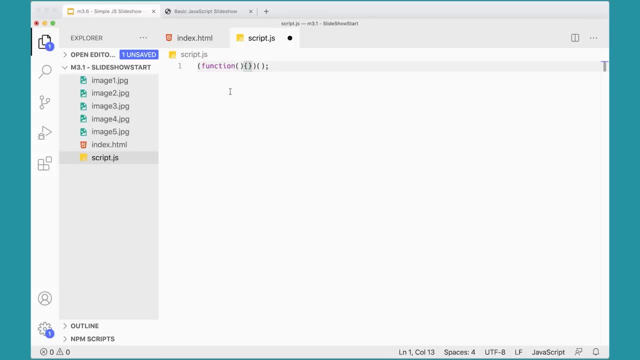 with other things. perhaps you've got other things going on in the webpage. perhaps you've got other javascript elements going on in the webpage. you don't want current image to conflict with some other current image variable for some other script, so we want to keep everything inside. 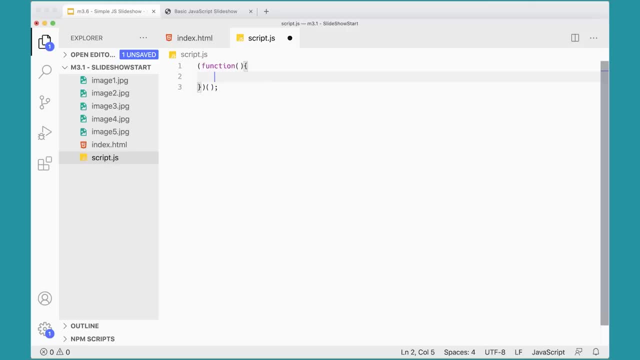 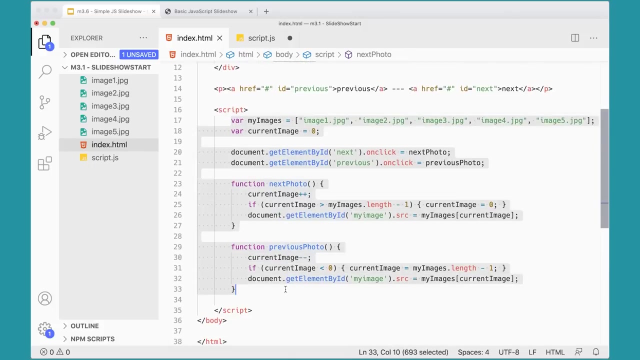 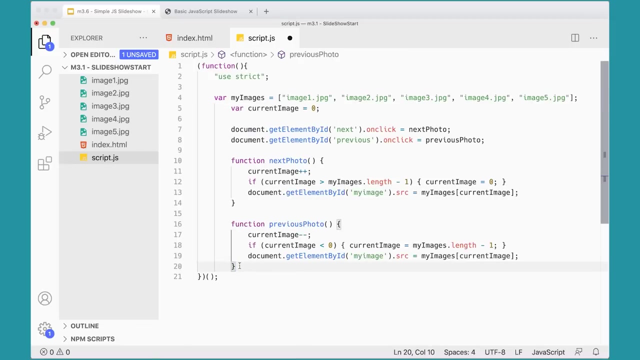 of this function. so I'm going to click between here and I'm going to also add my use strict directive and then in here I can just paste my entire script from here and there it is shift tab to move that back. and even better would be to replace these variables. 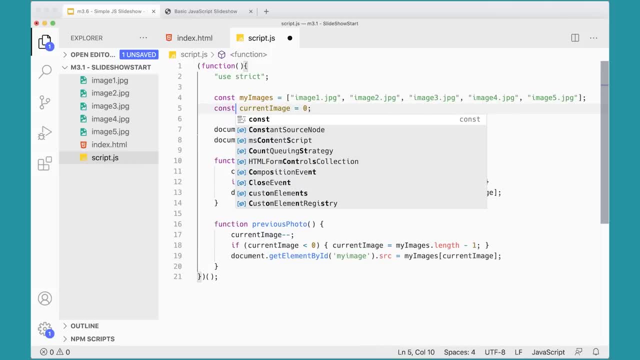 with const they're not going to change. well, actually, this one can't be const current image that one's going to change. that one needs to be let because current image is going to get reassigned as we go through our scripts down here. but these variables will now be. 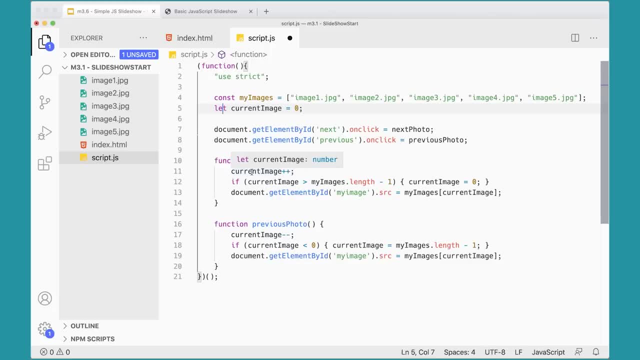 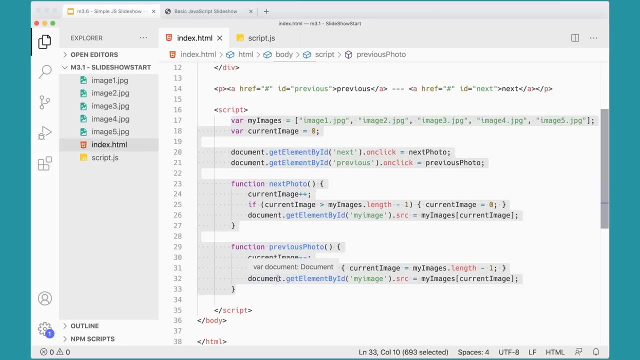 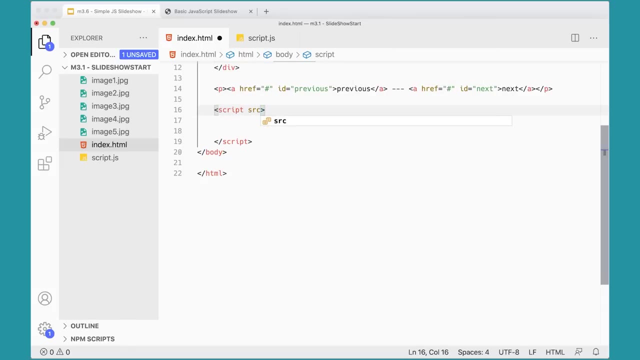 local to this function and they won't be available at the global scope. so we want to keep everything nice and tidy in the script here. alright, over here I'm going to remove that stuff and instead up here just link: src equals scriptjs. even pops up there in my menu. 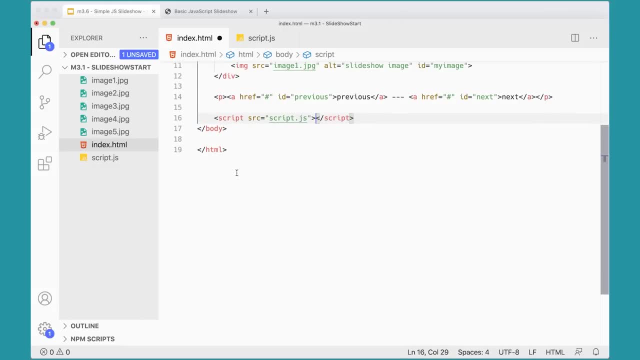 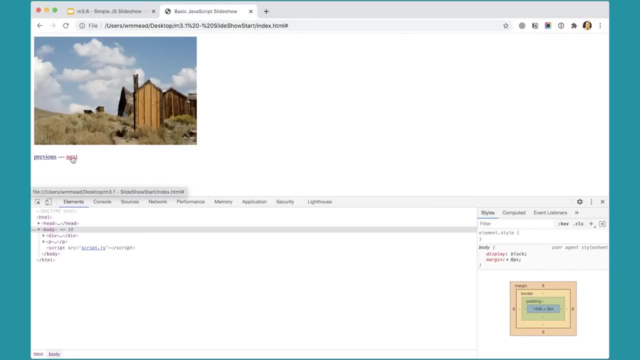 and I still need this closing tag, but I can move it up there and that should work just as well. we should go back and test it and make sure that we didn't make any mistakes in the process of moving stuff around, and you can see that it still works. 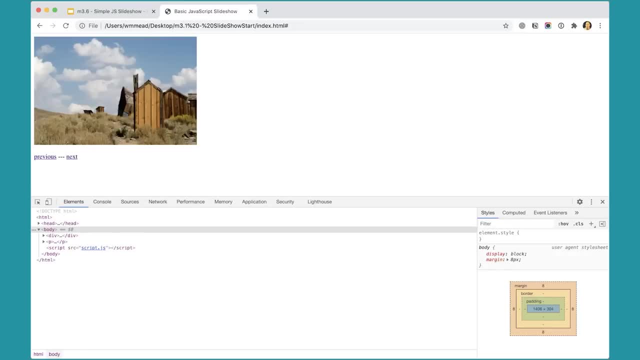 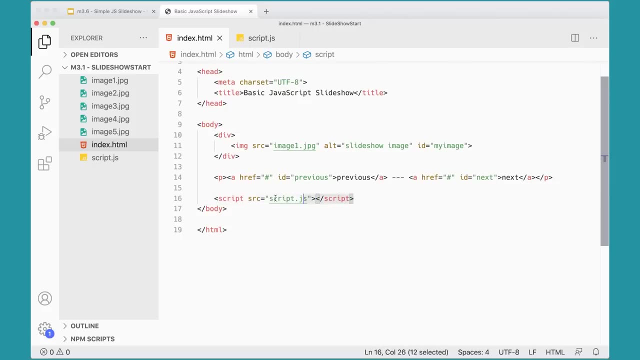 just exactly the same as before. now we could leave the script here at the bottom of the page. there's nothing wrong with that, and frequently I leave my scripts there. but even better is to move it up into the head of the page and add a defer attribute. 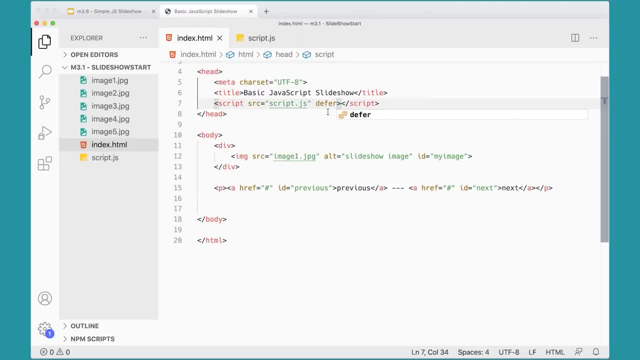 here. that will make the script load after the rest of the page is loaded and it keeps it out of the body of my HTML, which I really want to keep my HTML as clean as possible so it's easy to read, easy to understand, easy to update. 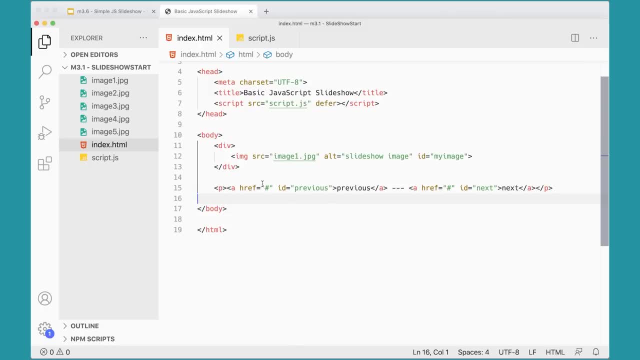 easy for Google to crawl. all of those reasons. I want to keep my HTML as clean as I possibly can, without any extra attributes, without any extra code or anything else. but once I've got that all in there and working well, I should always come back and just test and make sure I did it right. 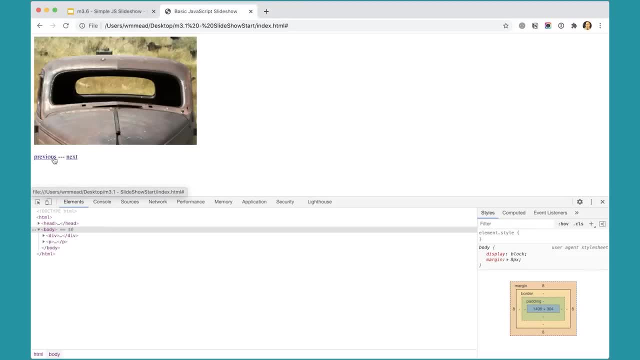 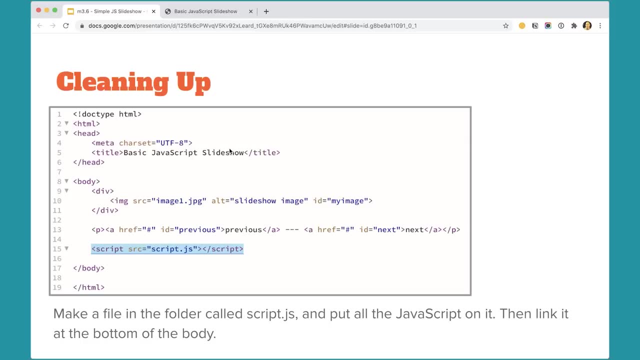 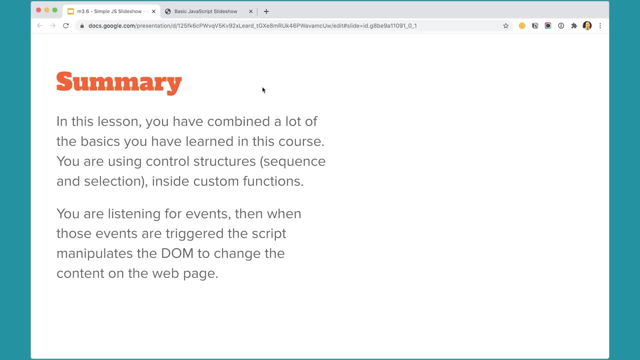 next previous, and that's working just fine. so with that we have a really nice script that's all set up and working well, and in this lesson we've combined a lot of the basics that you've learned in the course. we're using some control structures, such as the: 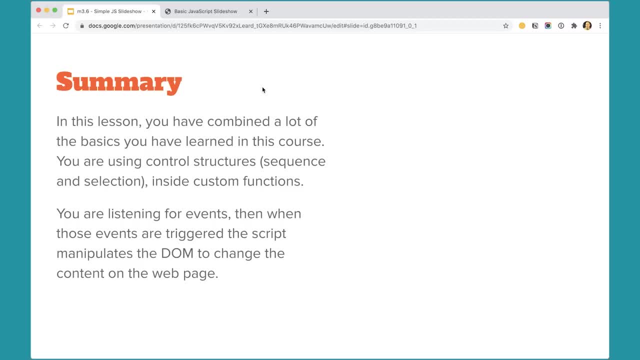 sequence and selection. we don't have a lot of loop in this one, but we're using sequence and selection. we're using the custom functions. we've got event listeners. when those event listeners trigger, we're affecting the DOM to change the web page. so all of these. 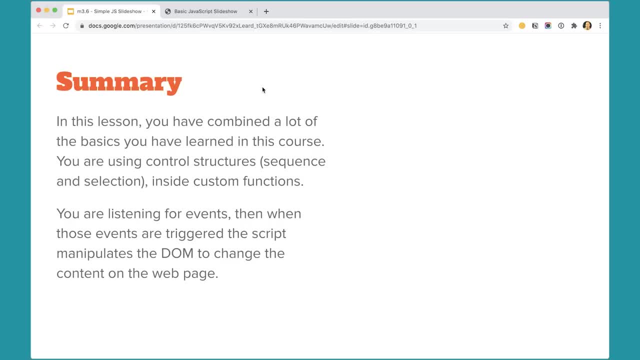 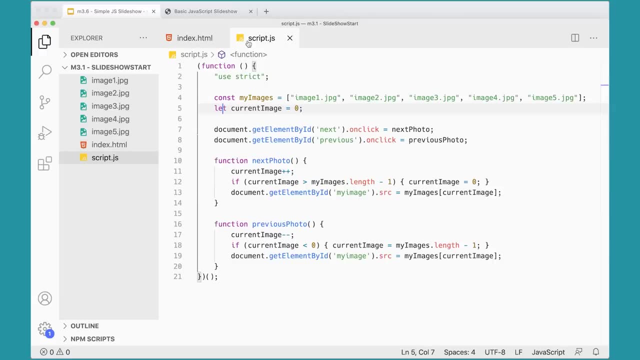 things are going on now. what you could do to make this script even better, perhaps, or just to test what you know so far, is go back to the script, and how could you replace using the one click event handler with using the add event handler method instead? and 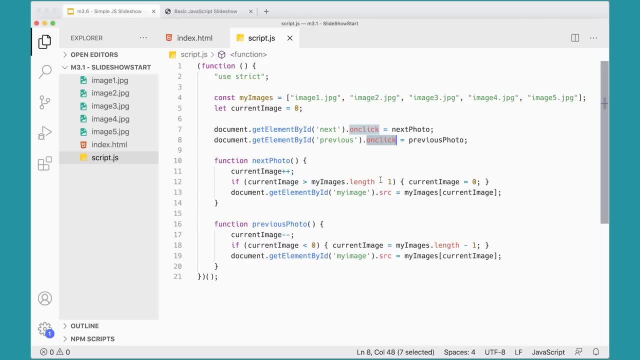 I recommend giving that a try, because that's a really good challenge to see if you can figure out something on your own without making it too hard, without going too far. so see if you can do that, because that will really be to your advantage. okay, great, great job putting this. 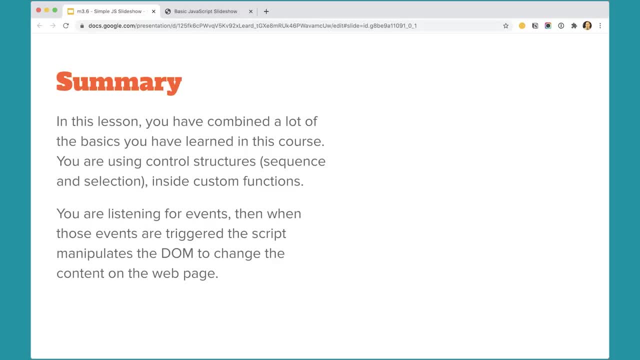 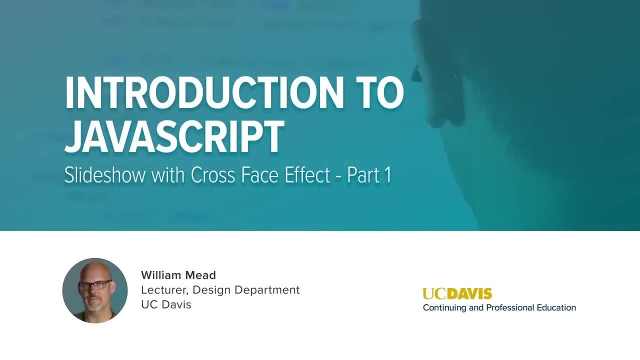 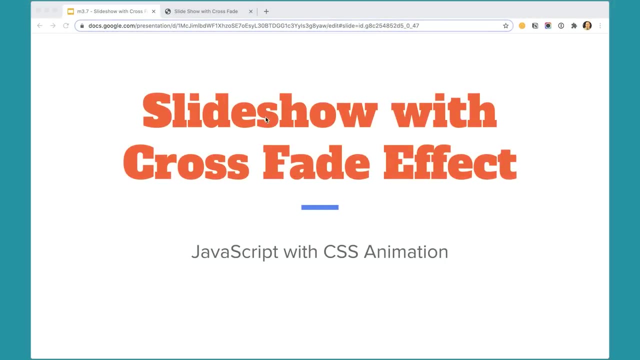 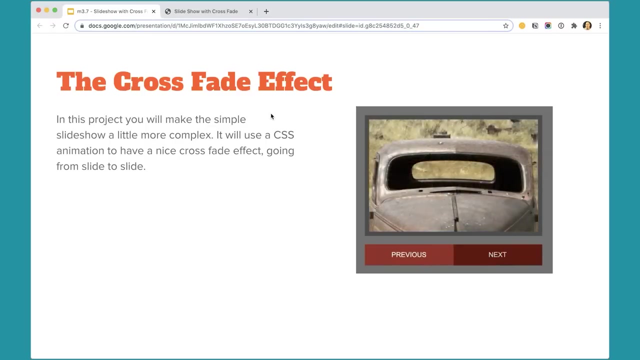 together and we'll see you in the next lesson. slideshow with cross fade effect. JavaScript with CSS animation. for this version of the slideshow, we're going to do something very similar to what we did before, but with a little bit of a twist. it's going to be: 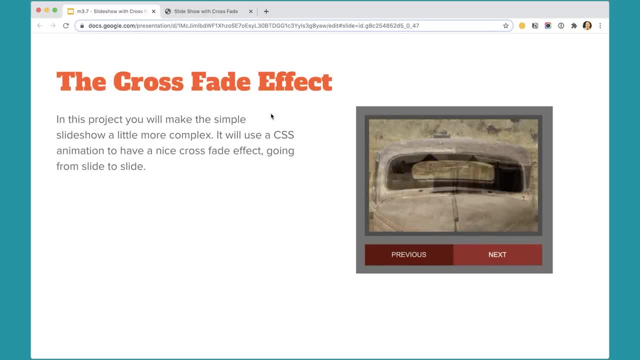 a little bit more sophisticated and I've got a little styling in here to make the slideshow look a little bit better. but instead of just swapping out the source, we'll have a cross fade effect as we go from one slide to the next, and we'll be using 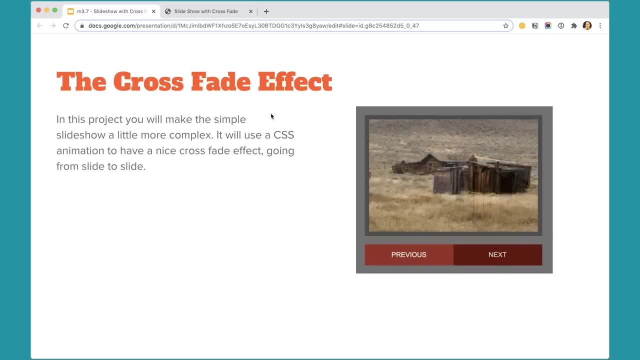 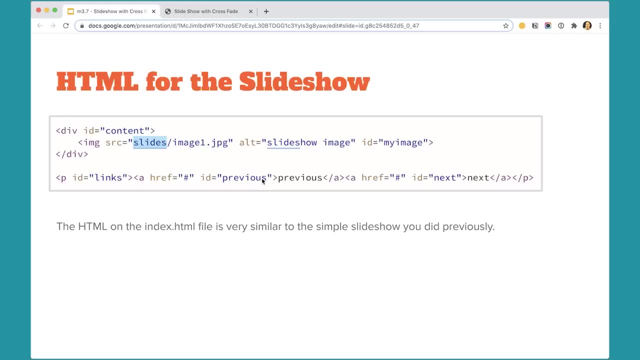 CSS to do that animation, so it's going to be a little bit different than what we did before, but very similar otherwise. the HTML for this slide deck, for this slideshow, is very similar to what we had before. we just have images, but now I have a folder. 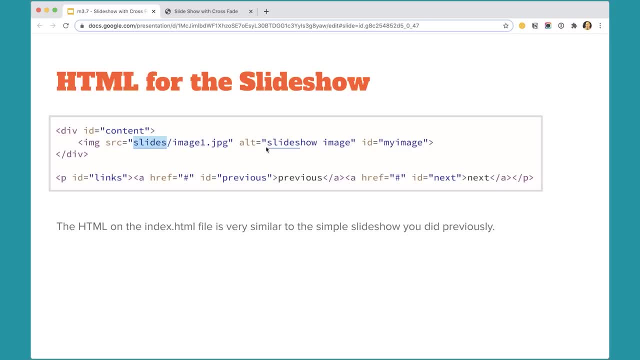 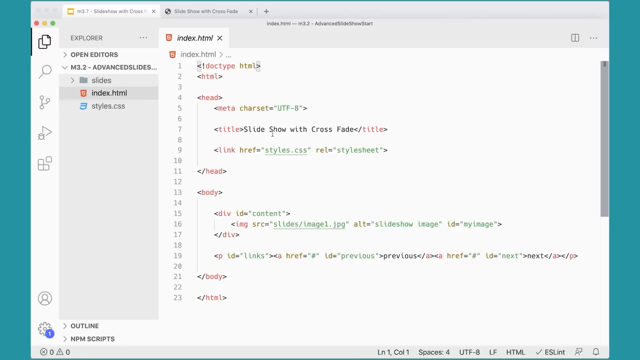 called slides. so image source, slide, image one. and then I've got an alt tag and the id for the image here and then I've got my next and previous links, as I had before, and you can see that over here in my HTML. so very simple setup with an image. 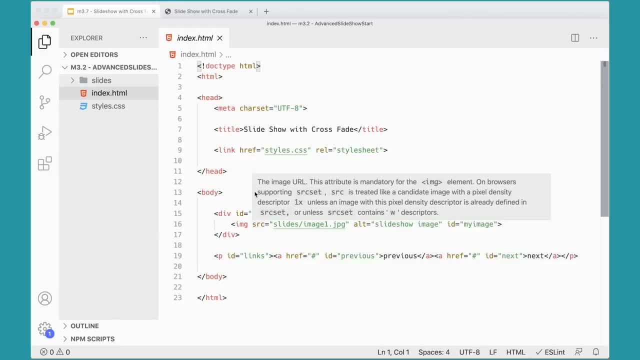 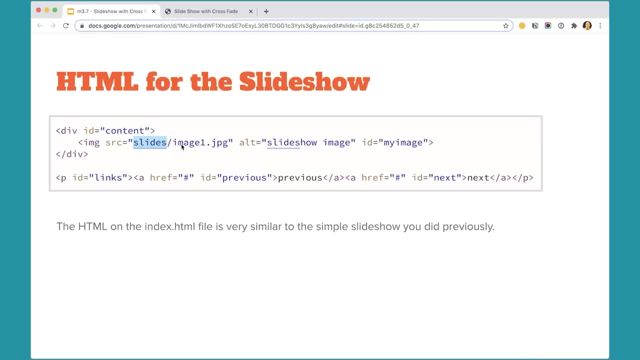 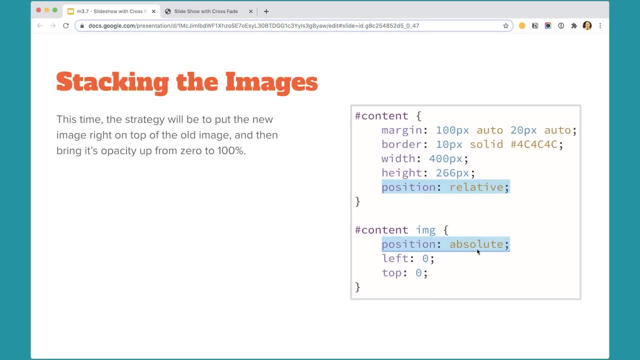 inside of a div called content. one thing that's different is that this time I'm using CSS to create to tell that content to be positioned relative, and I'm absolutely positioning these slides inside of here. so this content is set to 400 by 266 pixels, which is: 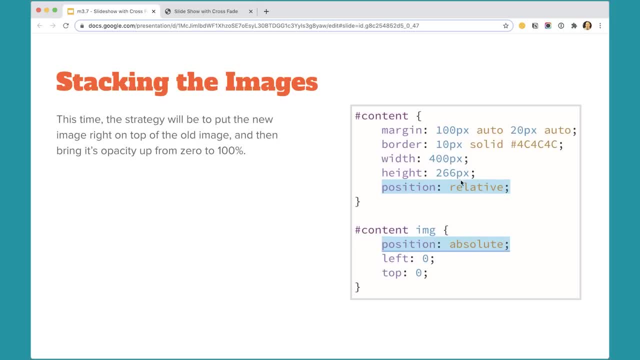 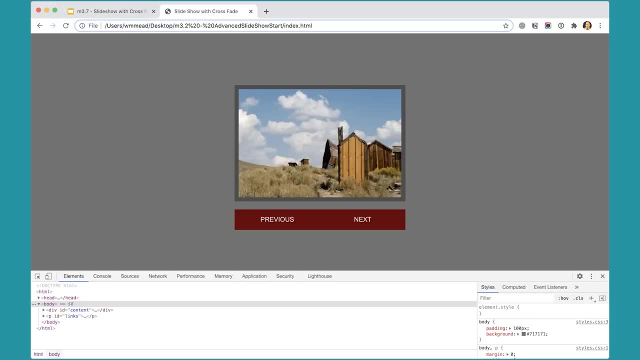 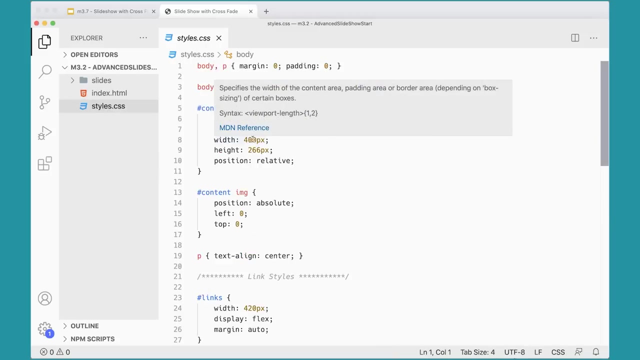 the exact size of the images that I have, and over here you can see it here on the page. now. if I were to go into my CSS over here and adjust that, you'd see a little bit better exactly what's going on here. so if I made this 500 wide, 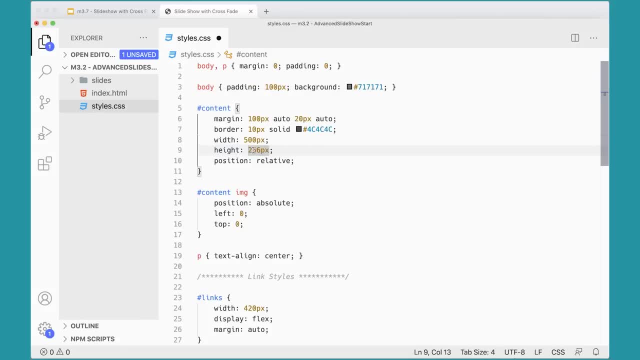 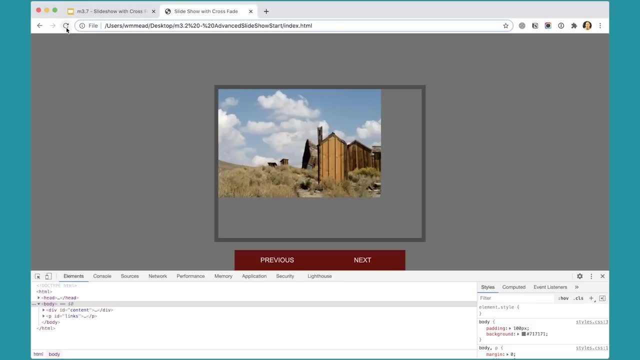 instead of 400 wide and 366 instead of 266, and save that. you'd see over here when I refresh this that the image is pinned to this upper left hand corner and before it was the same size as the box that it was in, whereas now 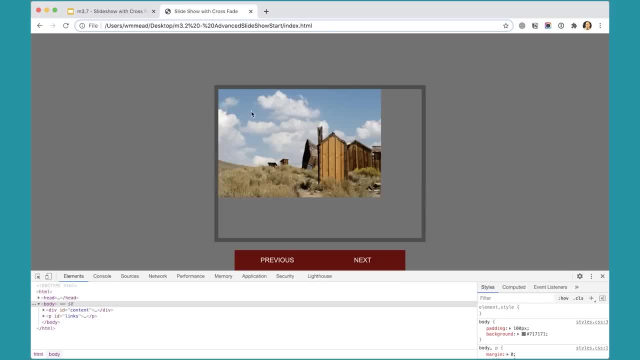 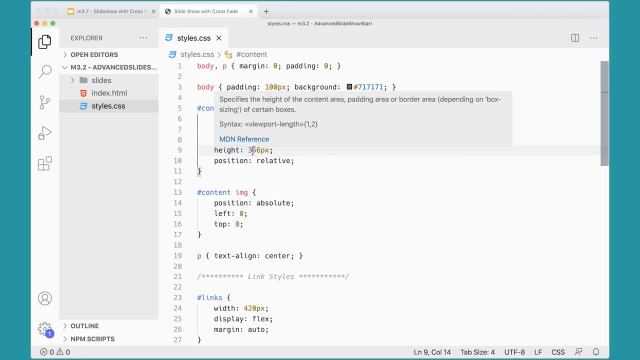 I've made the box bigger so you get this empty space up here, but the image is pinned up into the corner and it's important to understand that, because the way this slideshow is going to work is we're going to put a new image right on top of the old. 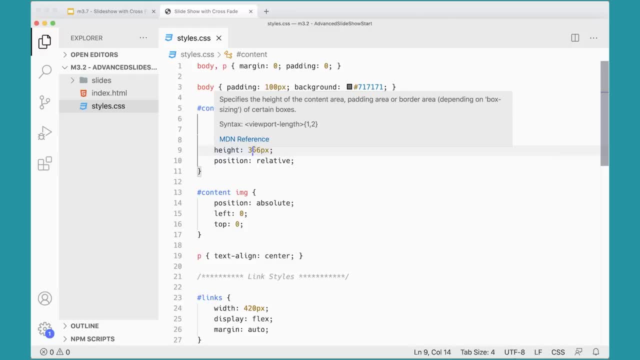 image and then we're going to cross, we're going to put it in fully transparent and then we'll fade it in so that we'll use. so you'll get that cross fade effect. but you can see the image. here is position: absolute: left zero, top zero. 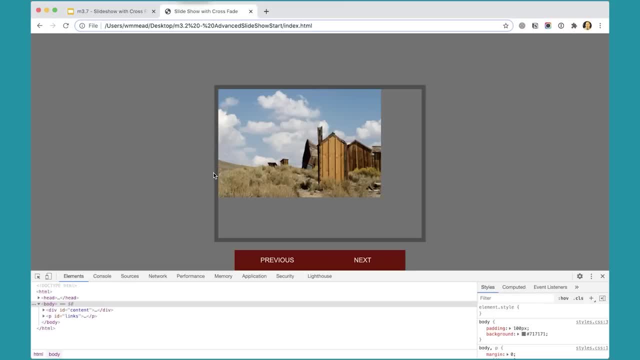 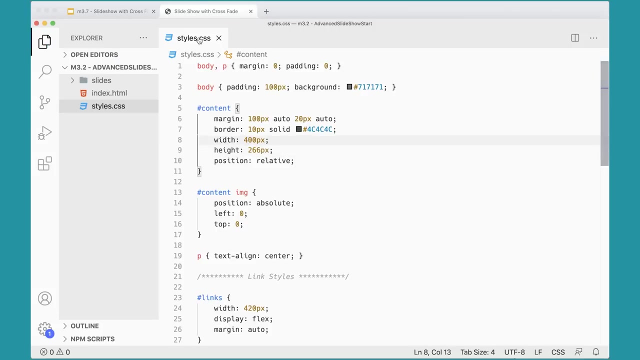 so that's what's putting that image inside this parent element, this container at the top left corner, left zero, top zero, and that's what's going on there. so we can put these back, because that's just for demo and you'll see if I refresh this that. 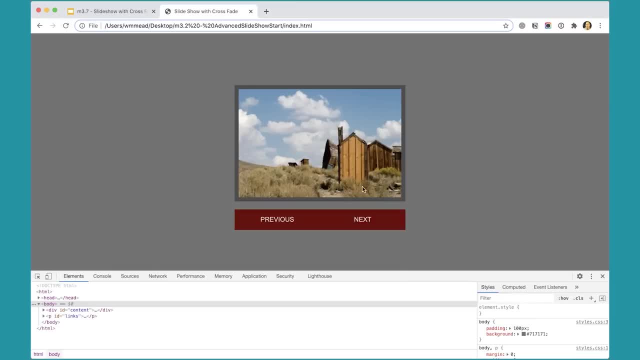 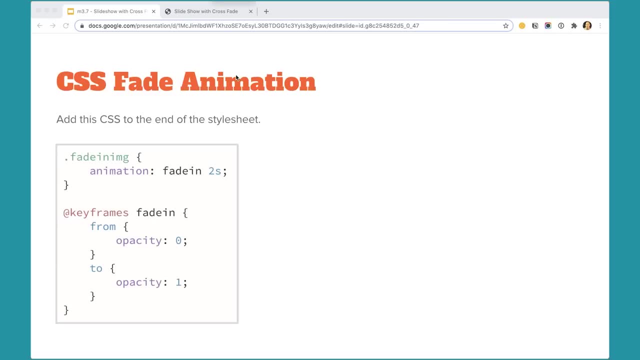 the image is now once again fitting inside that box perfectly, so it's important to understand that before we start with this. the next thing we need is the actual CSS animation that's going to actually do the cross fade effect, so we need to add this to the style sheet. 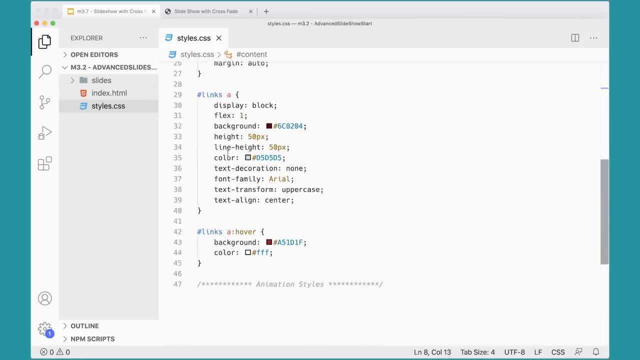 so go back to visual studio code and on the styles down here at the bottom, we can add these animation styles. so I'm going to add a class called fade in img, fade in image, fade in image. and what is that class going to do? it's going to 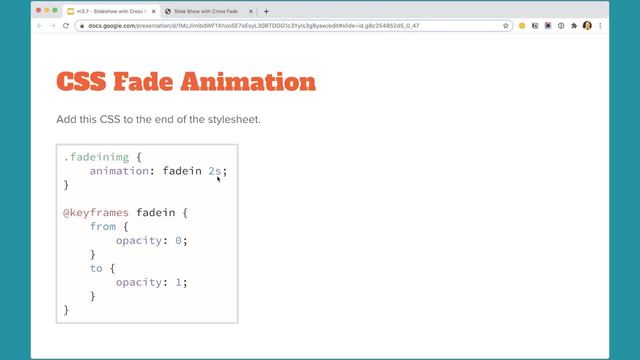 come over here and see here we're going to run an animation called fade in over two seconds. two seconds is kind of slow. you can make it one second, you can make it even slower. I'm making it kind of slow so you can really see it, see it taking effect. 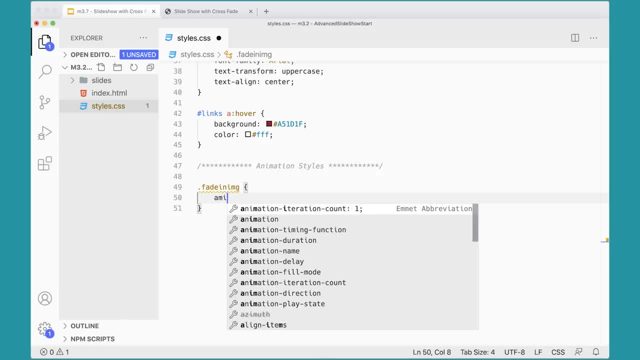 as we do this- but you could make it run a little bit faster- animation. and then we want to do two, we want to do fade in over two seconds, and that's fine. and then down here we're going to have, we're going to have a function. 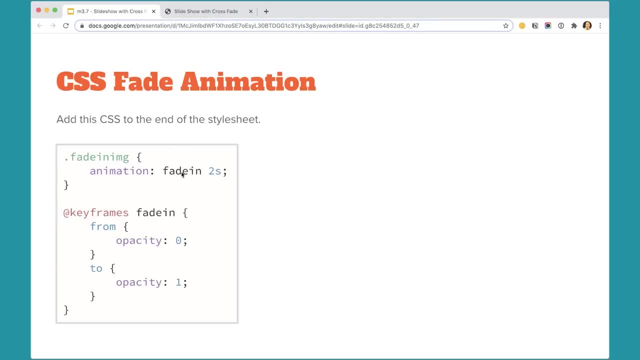 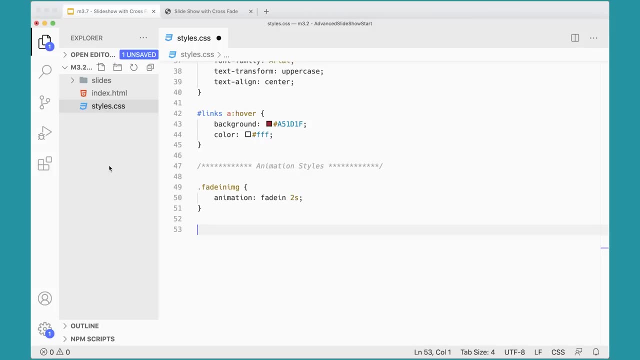 that will allow us to fade it in in that keyframes function called fade in. so these two names have to match. so we'll add at keyframes fade in, fade in, and then we're going to go from opacity zero. so we'll do. oh, I forgot from. 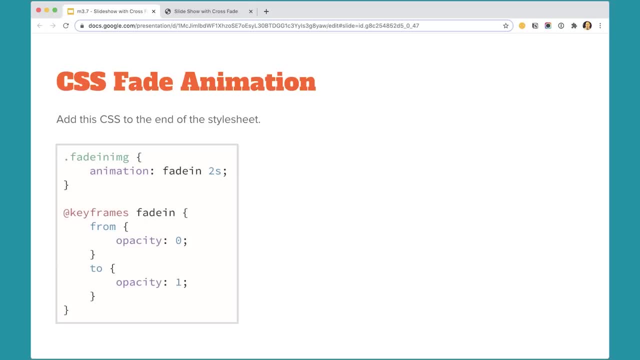 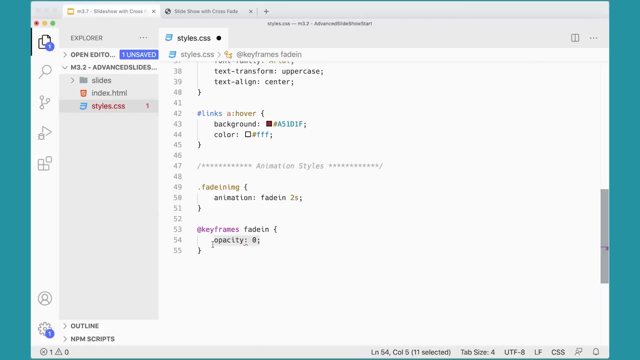 from opacity zero to opacity one. so it's a very simple animation. you can make much more complex animations using this fade in: from opacity zero, opacity two, opacity one, opacity one, opacity. okay, great, make sure you save this file. it's got the dot up here, so make sure you save. 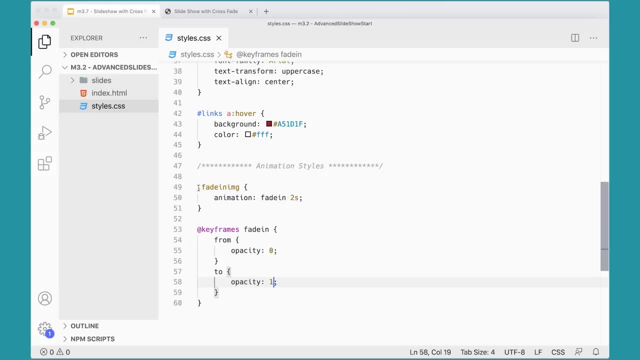 the file. so you've saved that and make sure you have this in here correctly, because we're going, when we add an image on top of the other one, we're going to add this class to it and then this class is going to run this fade in at keyframes. 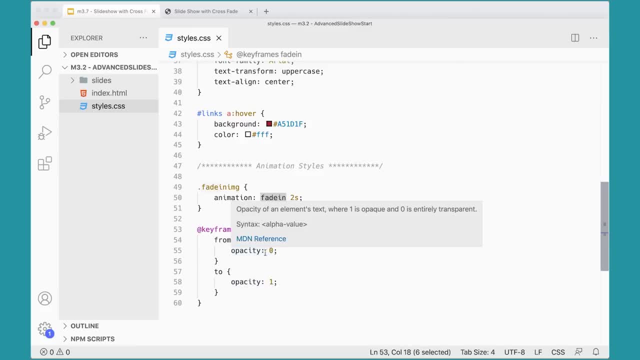 fade in here, which will start at zero and then go to one, so it'll come in at completely transparent and then fade into one which is completely opaque over two seconds, and that's what's going to actually create that cross fade effect. so none of this is being 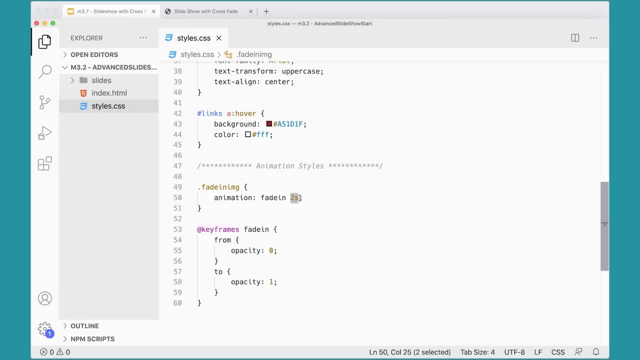 done in javascript itself, and that's actually great because you can do this kind of thing in javascript, but it's much more efficient to do it in css. if you do it in css, then you can take advantage. the browser will take advantage of the gpu, the graphics. 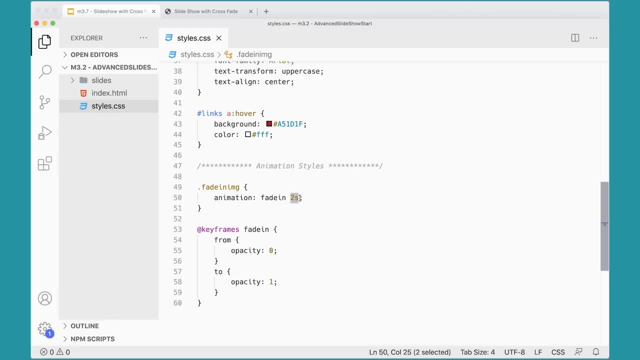 processing unit of whatever computer or device you're using, whereas if you do it in plain javascript, it's just the normal cpu and the gpu is really optimized to handle this kind of thing, so it'll be nice and smooth and work much better if we can do the actual. 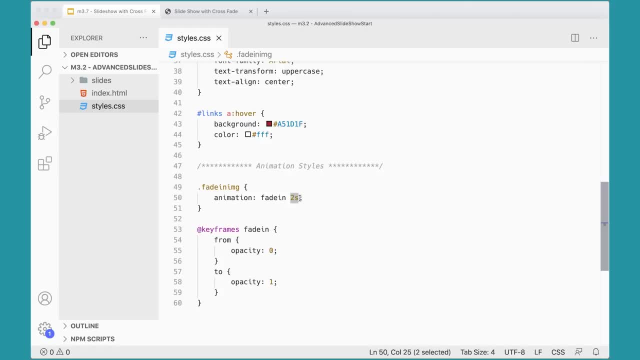 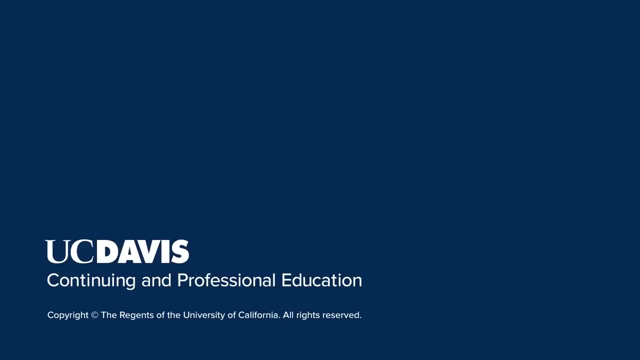 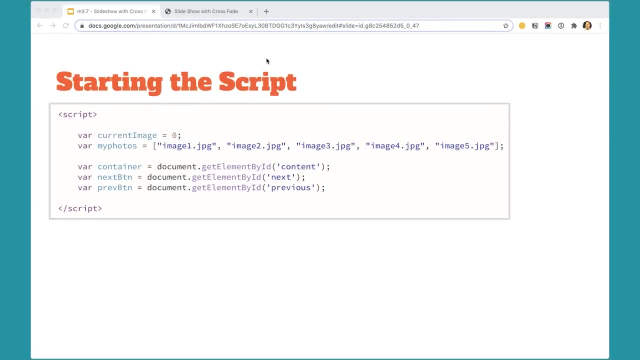 animation in css and we're frequently going to do that with javascript, where we use javascript to trigger css animations. and although we can do the animations directly in javascript, whenever we can use it to trigger css animations, it's better for performance across all kinds of devices. now we're all set up and ready to go. 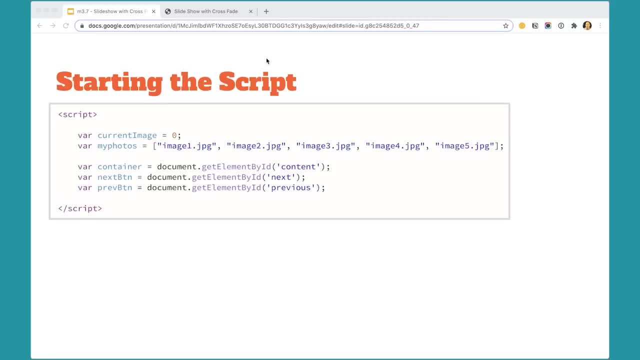 and ready to start writing our script. and our script is going to start with just a basic um variable, again for our current image and our array, same array that we had before, same current image variables. and then i've got variables for the container which is going to go get that container that we 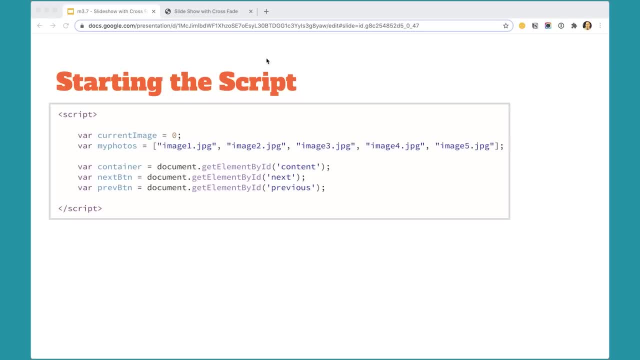 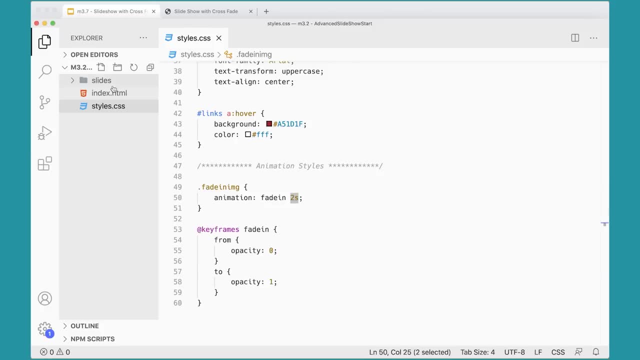 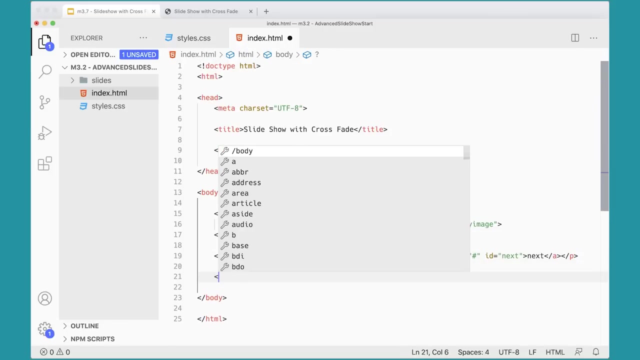 that's holding our image, and then for the next and previous buttons as well. so let's go ahead and get these set up in our script. so, going back to our index file, here i'm just going to add script tags at the bottom of our script. here our 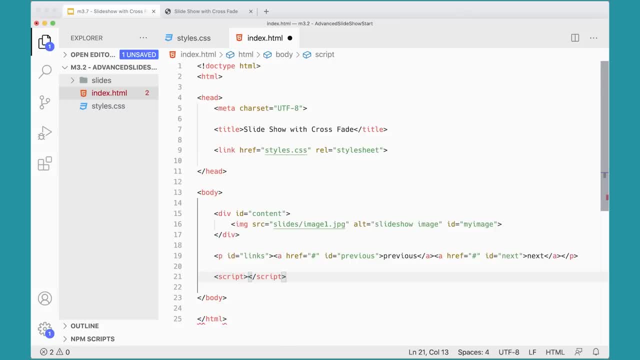 html script like so, and then i'm going to add a var current image and i'm going to set that to a value of zero initially, and then i'm going to have var um to do to do. i want to make sure i match the same name that i have. 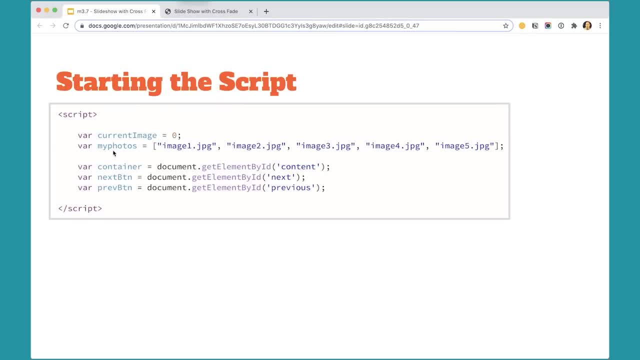 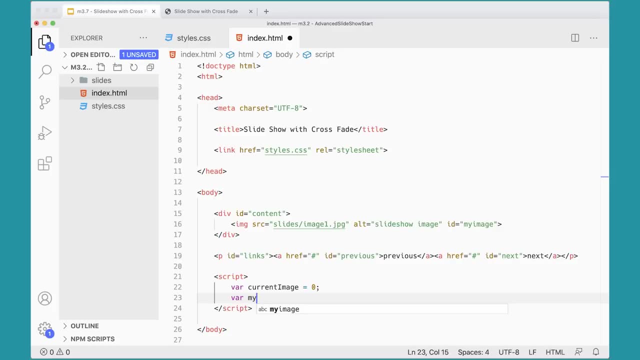 over here, call it my photos. this time i used a lowercase p, so make sure you watch out for that. if you want to make it match, my slides, my photos, equals. doesn't matter if it's a lowercase p or an uppercase p, but you want to make it match and. 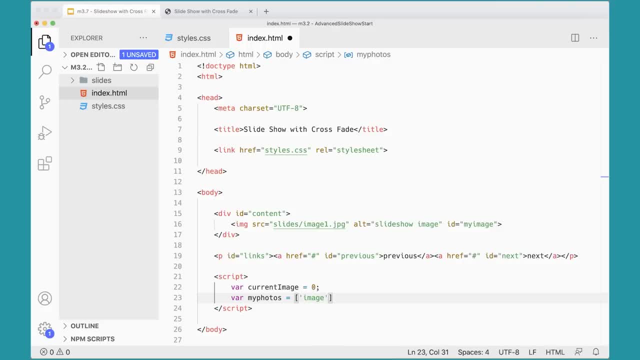 as before, we're going to have our array image: one dot jpg, um comma space, and then i'm just going to copy this. and again, it doesn't matter if you use single quotes or double quotes, probably best if you're consistent, but doesn't really matter. three: 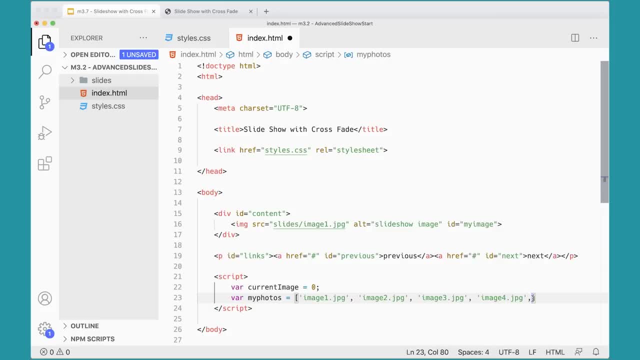 four and five. and remember, for the last one you don't have a comma, so you want to get rid of that comma, to add a semicolon after this array here. a lot of times when students are typing these at first, they forget that each one of these 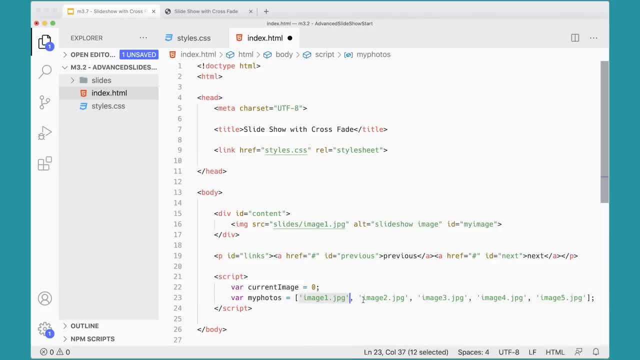 needs to be inside a set of quotes. so make sure that you've got each one of these inside a set of quotes, followed by a comma. you can't just add a quote here and a quote at the end and then put them all in there with commas. you have to have each one. 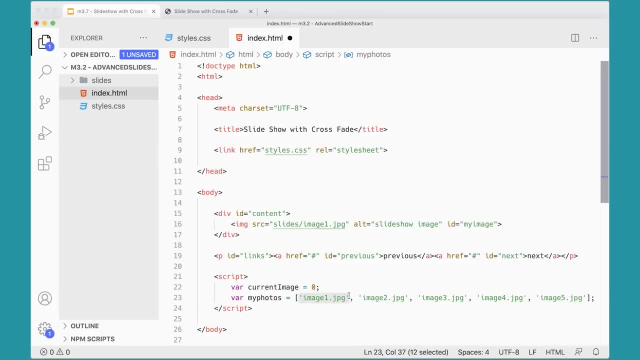 is inside of a set of quotes. okay, so we've got that, and then the next thing we need are to get some variables: var. um container equals document dot. get element by id, and the id that we're getting again is this one content, and it's always good to copy and paste. 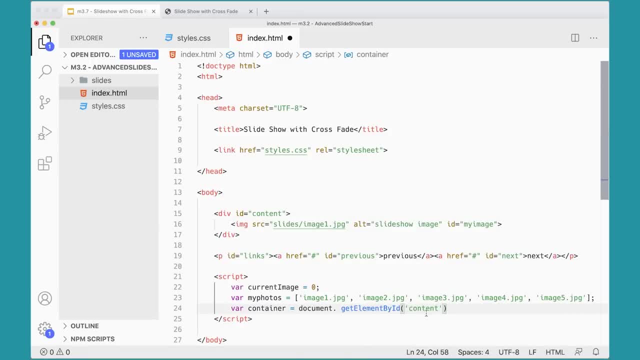 so that you don't spell that wrong. so that's going to get us that element. we also need the next and previous links. var next- btn- equals document- dot. get element by id. next- btn- equals document- dot. get element by id. var prev- btn- equals document- dot. get element by id. 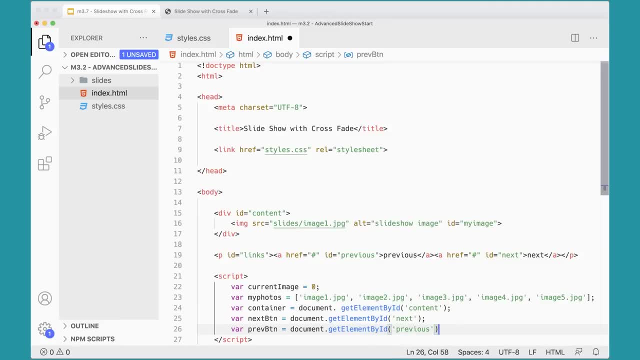 previous. so, again, that's going to go into our document. we're going to get our next button, we're going to get our previous button and we're going to get our our content div. that we're going to be adding here and i have an extra space there that i 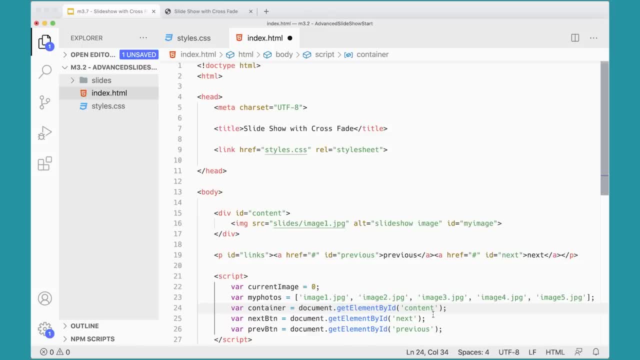 shouldn't have. make sure you fix that if you have that in there, okay, document. get element by id content: next and previous: great, so we've got all of that. in the next video we'll add the event listener for when you click on this next link here to go to the next. 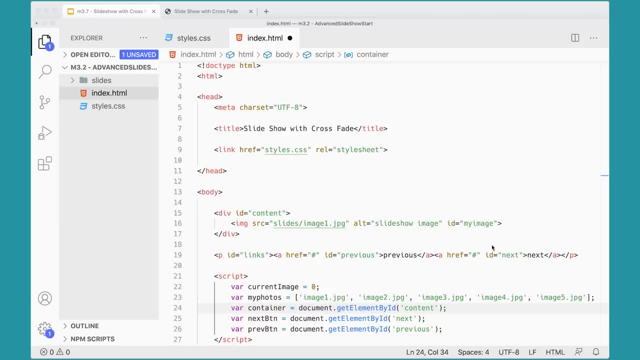 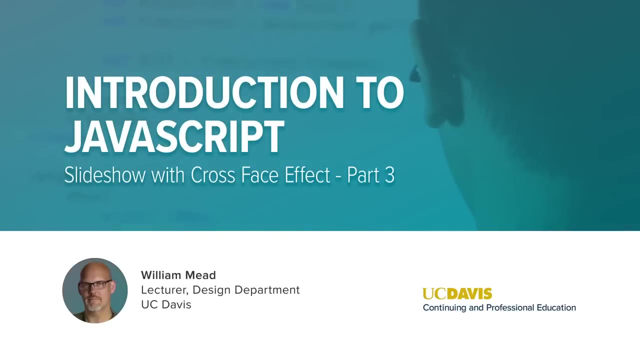 slide and, just like we did before, we'll build out the next one and then, when we're done with that one- we get that all working- we'll work on the previous one, so we'll go ahead and work on that one first. okay, here's our event, listener. 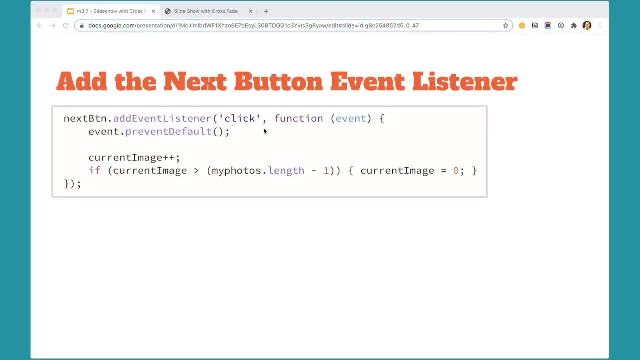 for when we click on the next, the next button, and for this one we're using the add event listener method instead of the on click property. so we'll look at this method and we're going to add the event listener right to that next button variable that we created. 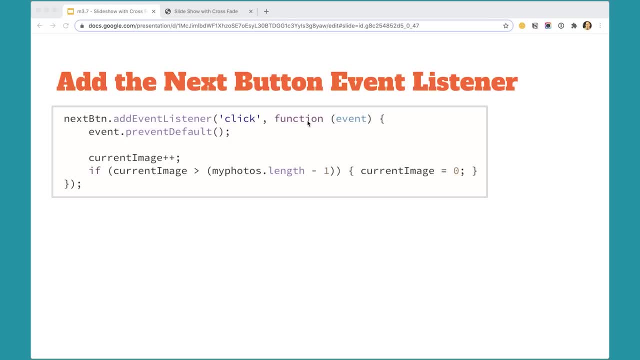 and when it's clicked, we're going to run a function- this is an anonymous inline function- and we're going to pass in the event object so that we can prevent the default behavior of what happens when you click the link. so we don't want to. really we don't want the browser. 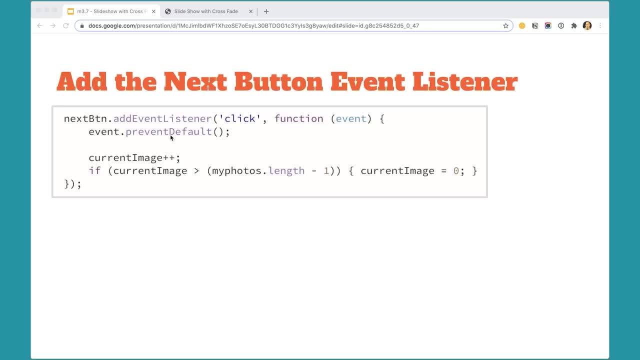 to handle clicking the links the way it normally would. we want to prevent that default behavior and prevent default. we'll do that when we pass in this event object here, so we'll prevent default and then, just like before, we're going to increment the current image and then we're going to check. 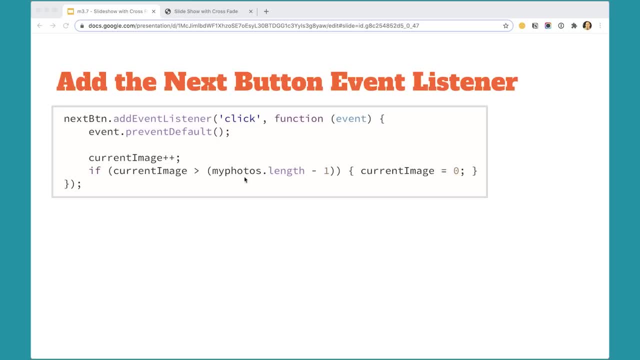 once again, if the current image happens to be greater than the length of the array, that we've got minus one. so again, this could be a four here, but instead of a four we're putting my photos: dot length minus one. if that's true, we're going to set current image back to zero. 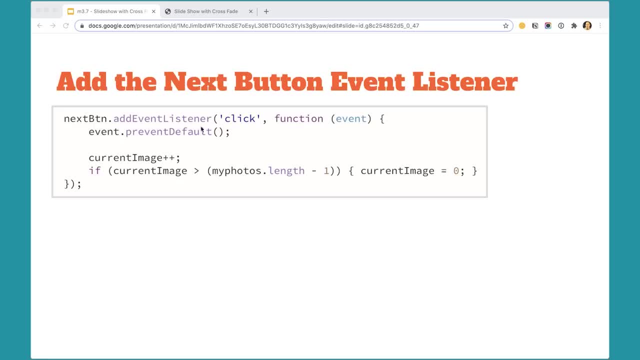 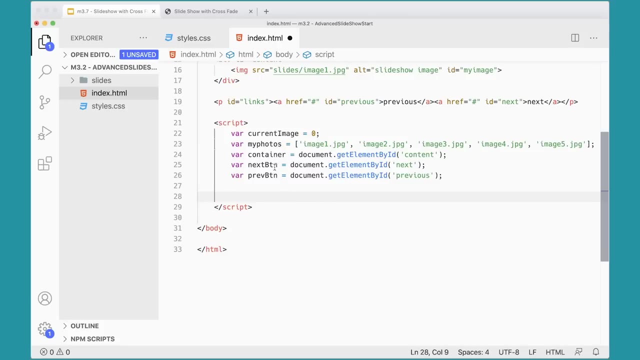 so that part's exactly the same as we did before, and really this part is only different because we're using the event listener instead. so let's go ahead and put this in. so i have my next button here, which is already going and getting that element, so now i can just do next. 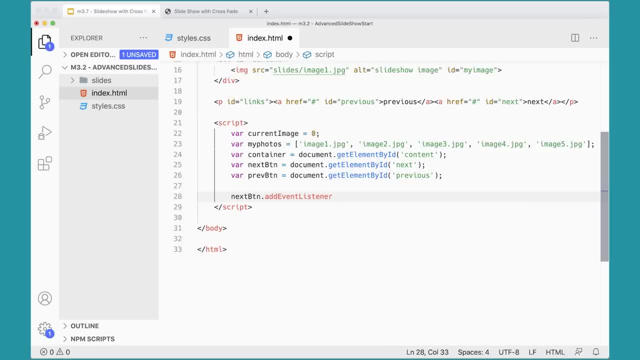 btn dot. add event listener and i'm listening for a click. that's what i'm listening for and when the click happens, i'm going to run a function and i'm going to pass into that function the event object and put a semicolon at the end of this. 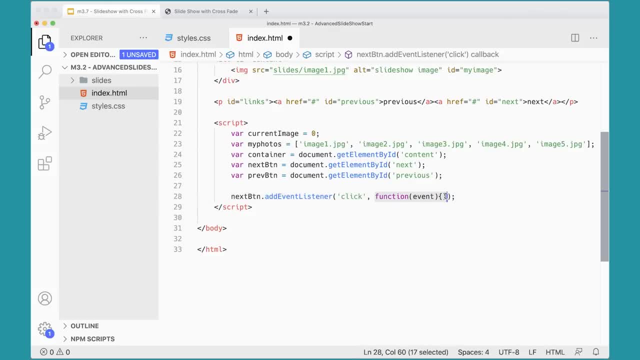 line. so this function is going to run when the click happens, and then i'm going to click inside here and i'm going to add something like event dot- prevent default. so that'll prevent the default behavior, so that when i click on this link i don't actually get the hashtag. 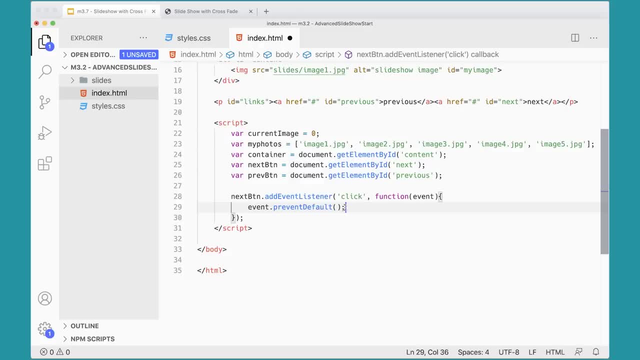 coming up in the browser and, um, that's kind of that's kind of nice to not have that show up. so it just prevents sort of even trying to go to this href at all, and that's great. and then what we're going to do is we're going to 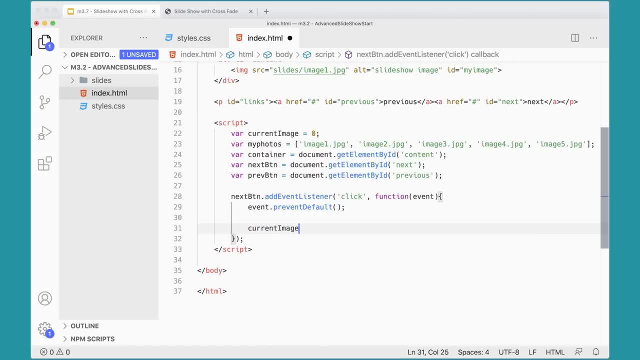 increment current image, current image plus plus same as we did before. and just like we did before, if, if current image is greater than my photos dot length minus one, so really a four, zero one, two, three, four. if it's greater than four, my photos length would be five. 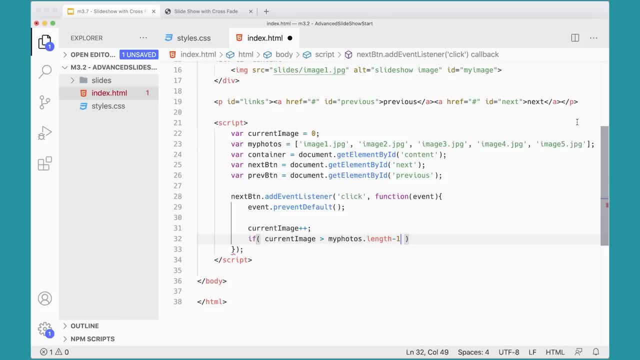 but i want to check to see if it's greater than four. if it's greater than four, then what i want to do is i want to move it back to current image equals zero, so i will put it back to where it was initially and again, you could put this on a separate line. 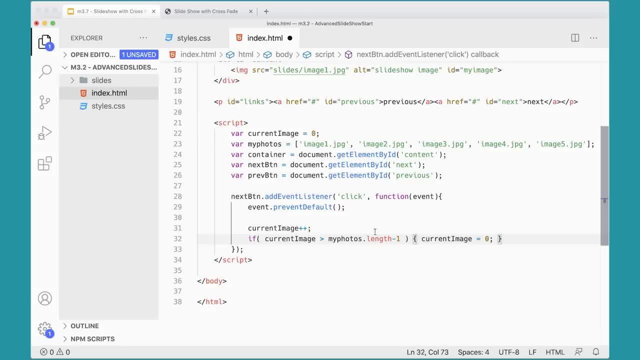 here. i kind of like it organized this way, because that's all just on one line there. there we go. so now current image is going to increment and it's going to go up and it's going to become, either it's going to go from zero to. 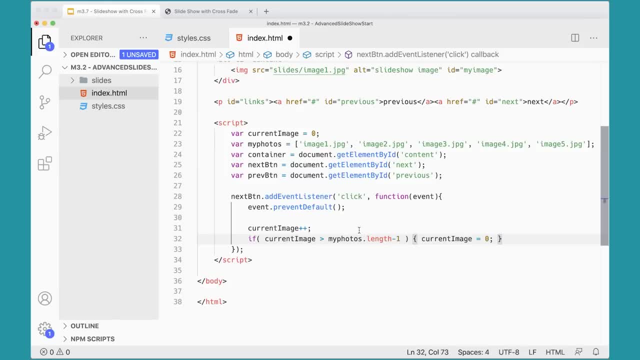 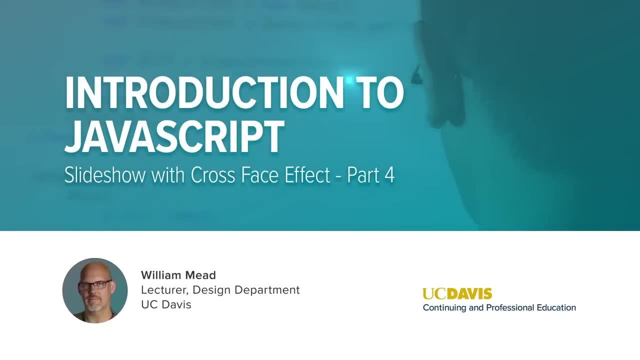 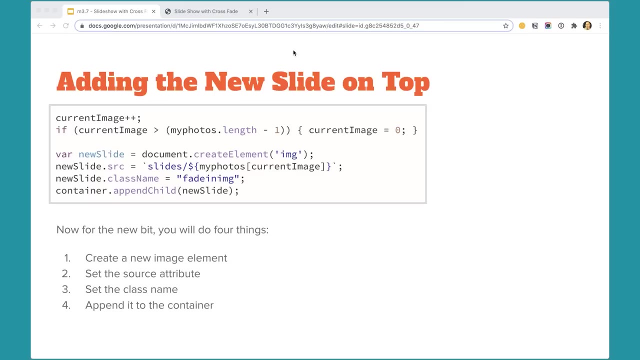 one to two, to three to four and then back to zero. here's the new part: instead of just swapping the source attribute, which is what we did in the first slideshow, in this one, what we're going to do is we're going to create a new image. 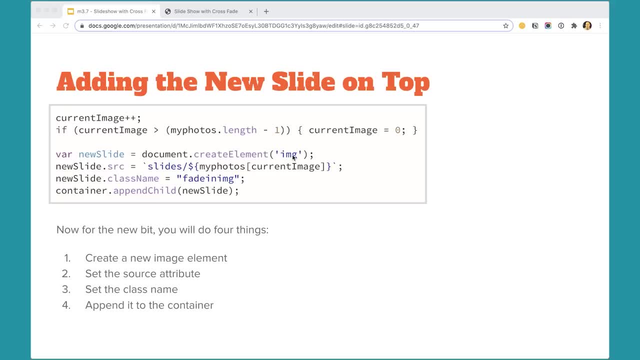 element document: create element img. so that makes a new image tag. i'm going to put it into this variable called new slide and then i'm going to set the source new slide src to slides slash. my photos, current image. notice the use of the tick marks here and 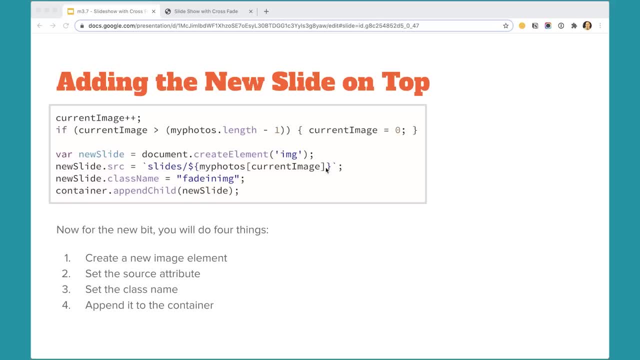 the dollar sign curly brace is going to hold the variable for the my photos thing. okay, so that's going to get. go get the next photo from the slides folder and then i'm going to also add a class name, fade in image, and you'll remember we just added: 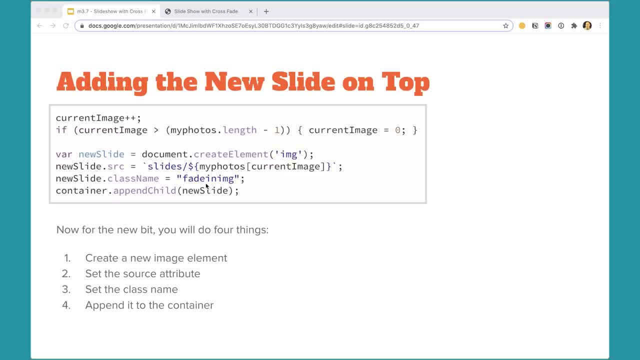 that class to the css, so we know what that does. when we add that class, it runs that animation over two seconds of actually feeding in the image and then we append the child to the slide. so the slide, so the the new slide gets appended to the container. it gets. 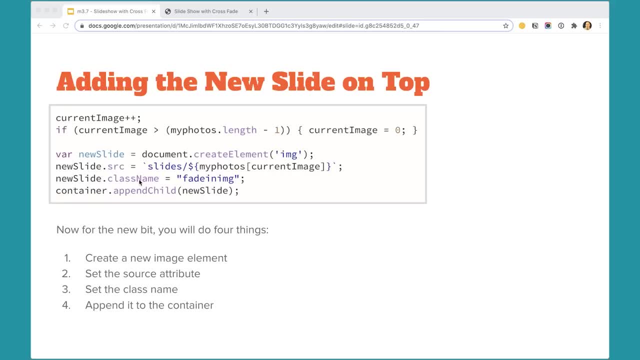 appended with this source and this class. as soon as it gets appended to the container, that animation runs and changes the opacity from zero starts at zero and it goes to one, which means it's going to go from completely transparent to completely opaque. and because we're adding it into this, 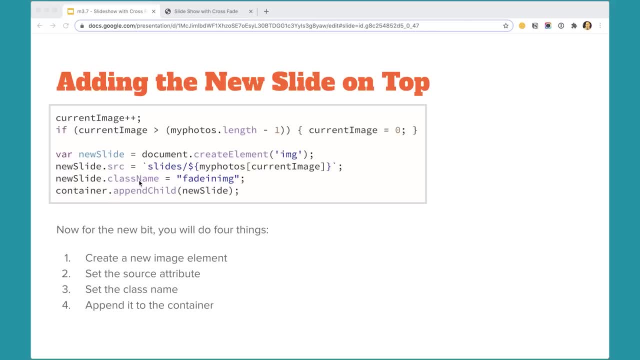 container and the css for that container is to make these images position absolute. it's going to get put right on top of the previous image and because it's the same size as the previous image, it will completely cover it, but because it comes in as transparent, you'll. 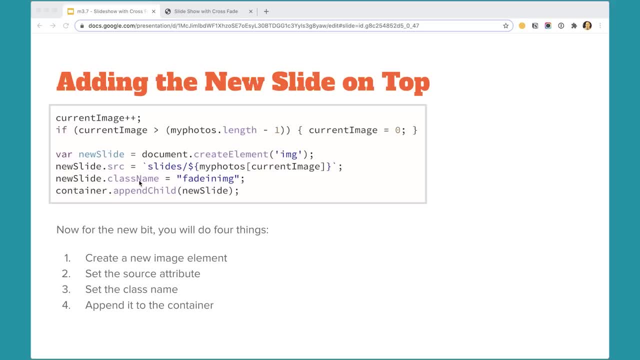 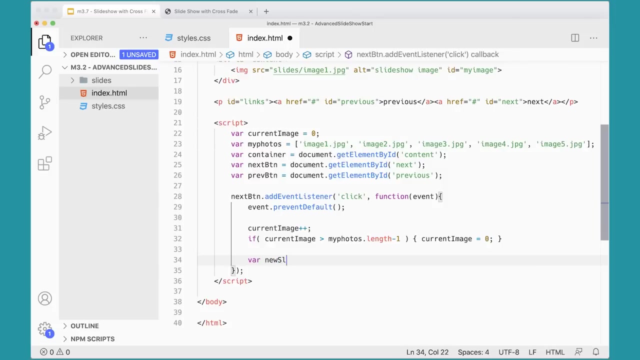 see the other image underneath it at first, and then, over two seconds, it'll become opaque and uh, and that's where it will cause the fade, in effect. so let's go ahead and add this to our, to our code over here, bar new slide, and i'm 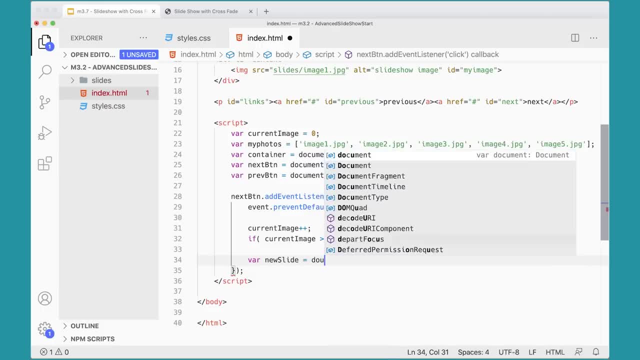 going to set that to document dot create element. and what am i going to create? i'm going to create an image img. so there we go. so now we've got a variable that's holding a new image element. the image element is not on the page, but it's there, and then i'm 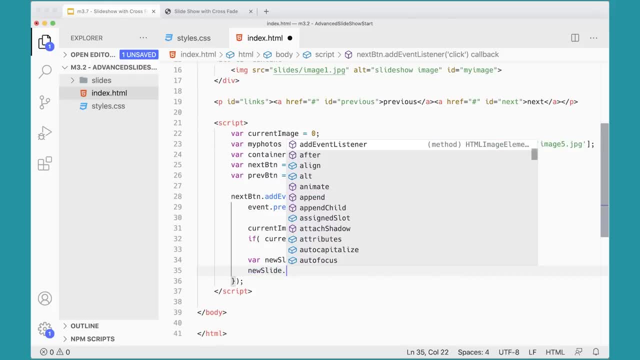 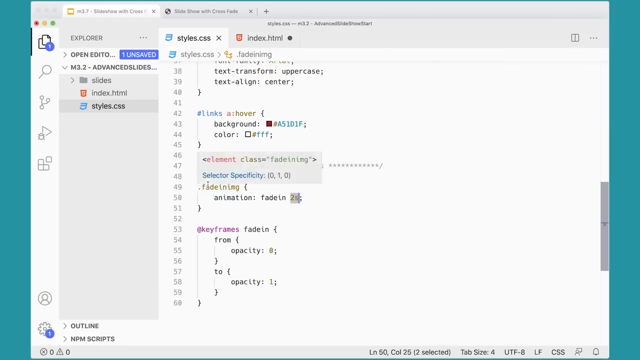 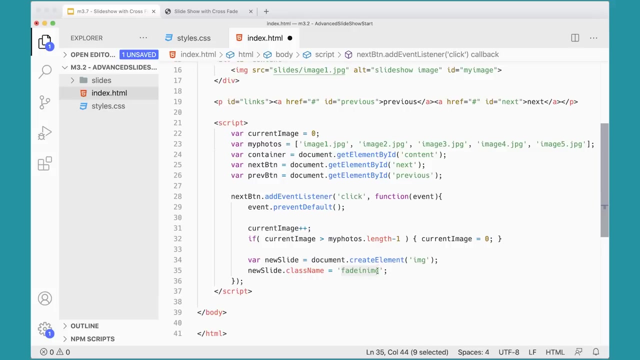 going to say new slide dot class name equals fade in img. make sure you spell it right. it needs to. this needs to match exactly what you have here: fade in image. those two things need to match. doesn't matter if if you spelled it differently from how i. 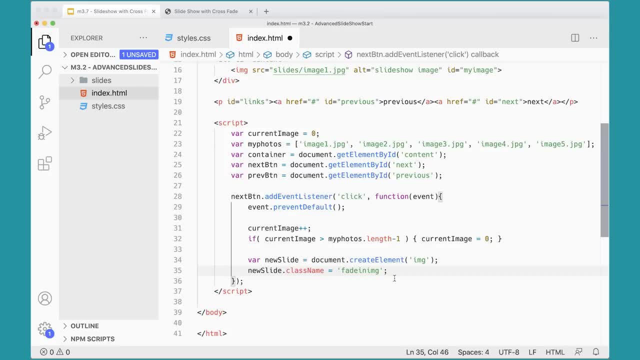 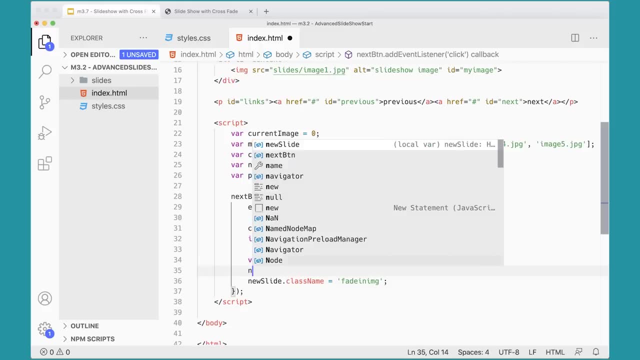 did. as long as this one matters, as long as they're the same as each other, and then that's fine. so we're going to add that on there. oh, i also forgot. i'm going to do new slide dot src. i'm going to set its source to: 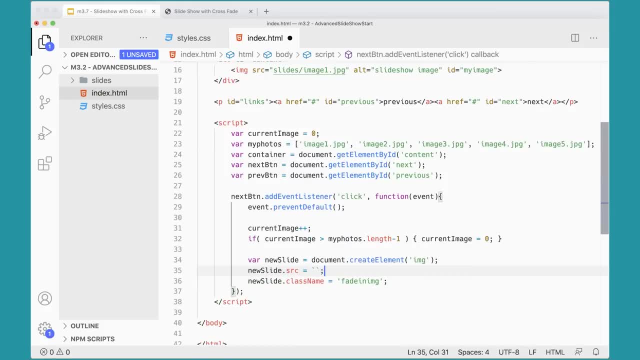 i'm going to use my tick marks here, tick, tick, and in here i'm going to say: okay, slides, because i'm in the folder called slides over here. i need to go to slides and then i need to do slash and i would put image one or image two or image three. 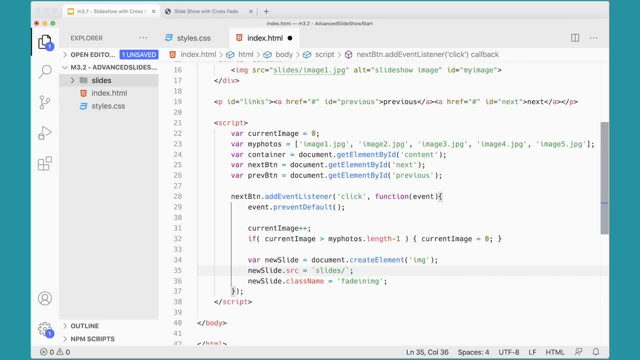 but instead i'm going to put a variable there. so again we do the dollar sign and the curly braces, so we can do a variable. and what variable do we want? we want my photos: square brackets, current image, that current image, right there, current image. so when we click the next button, the first time, 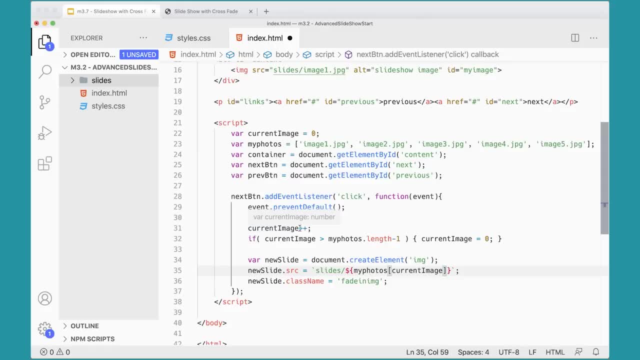 it starts off at zero when we click it the first time. it gets incremented to one. so when that gets incremented to one, a new photo gets created and the source gets set to. this gets incremented to one, so the source gets set to image two and that goes in there. so it's. 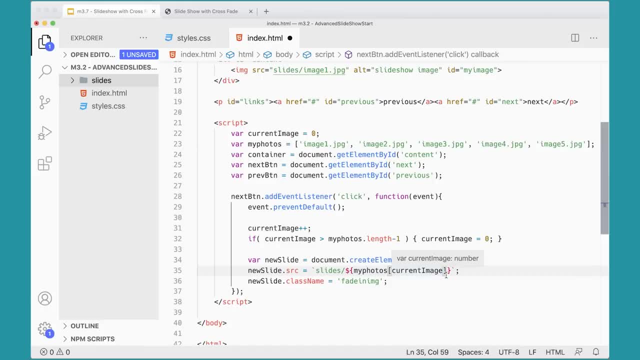 slide slash. that'll be an image two dot jpg the first time you click it. the next time you click it it'll be an image three, and when you get to image five, if you click it again, that gets beyond the length here, so it gets set back to zero. 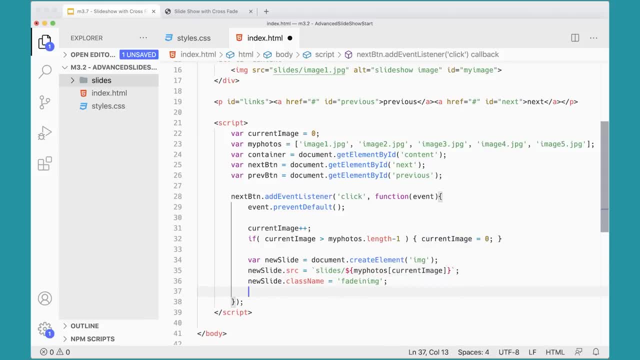 so it'll go back to one now. the last thing we need to do here is append this to the, to the container, and we created a variable here for the container so we can say container container dot. append child new slide. so it'll take that new slide that we created here. 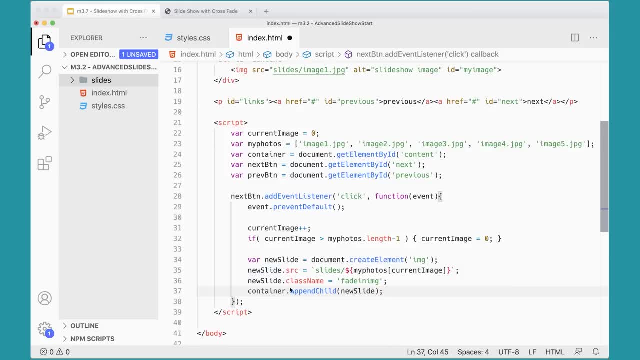 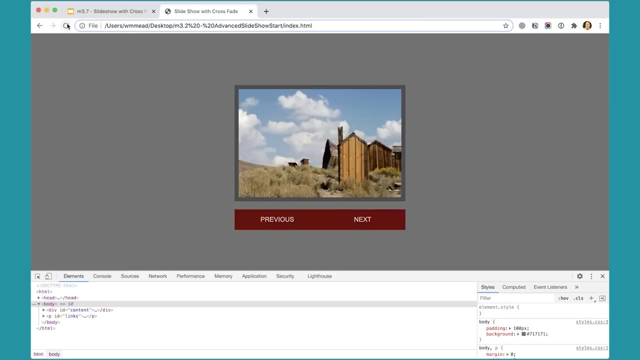 as an image, set the source, set the class and put it on in there, put it on the page. let's save this and see if i did it right. i'm going to go over to my slideshow here, click refresh and then click next and look at that. 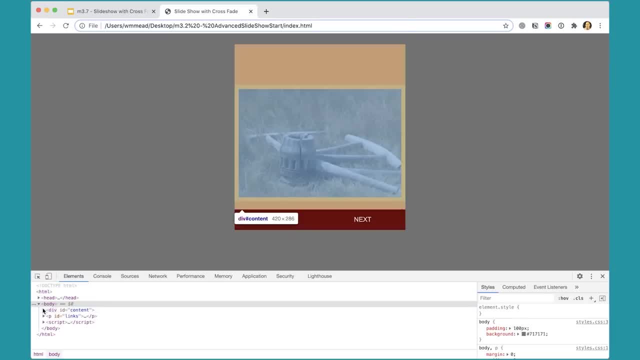 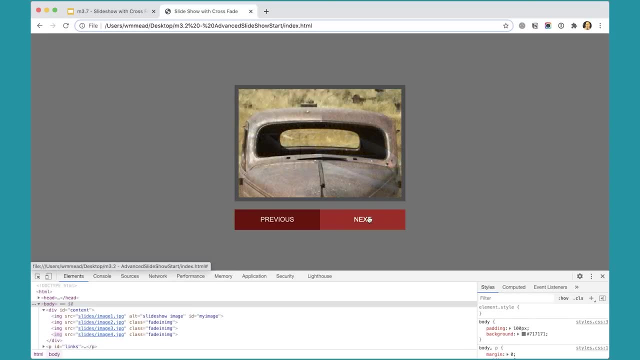 it's working. it's working just perfectly. next- and i can see in here that it's adding the images one on top of the other. it put three on top of two, it put four on top of three, it put five on top of four, and now it'll put one on top of. 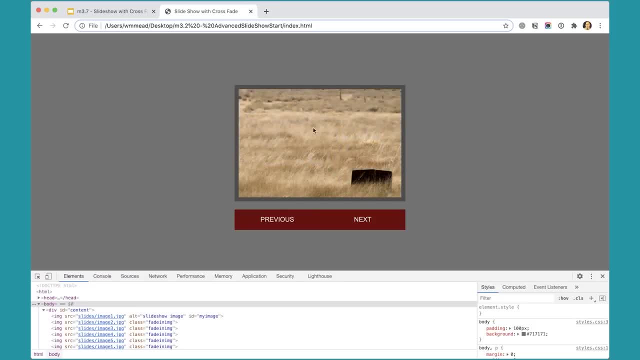 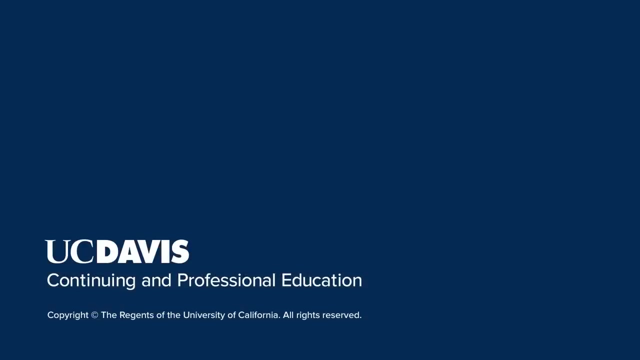 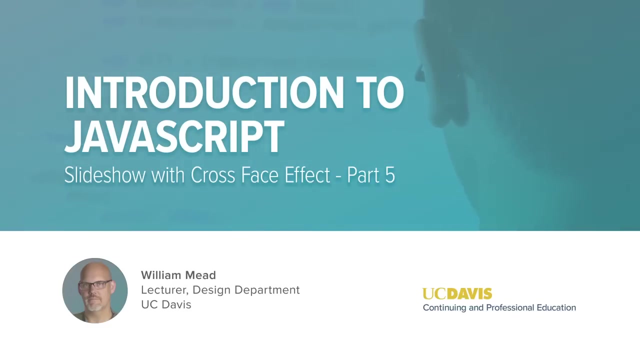 five and you'll see, as you're adding them, that animation is taking place. in over two seconds, the picture comes in as transparent and then, over two seconds, it fades to opaque, and that's what's creating that crossfade effect. as you just saw, this is working. 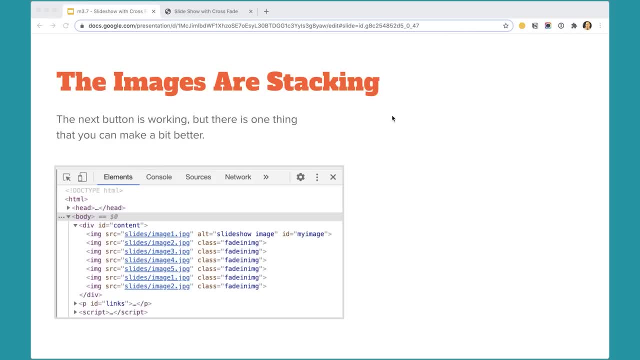 and the images are coming in and they're stacking one on top of the other and fading in. but there's one thing that we can do to make this a little bit better. i don't really like that. every time i click the link it's adding more images to the dom. 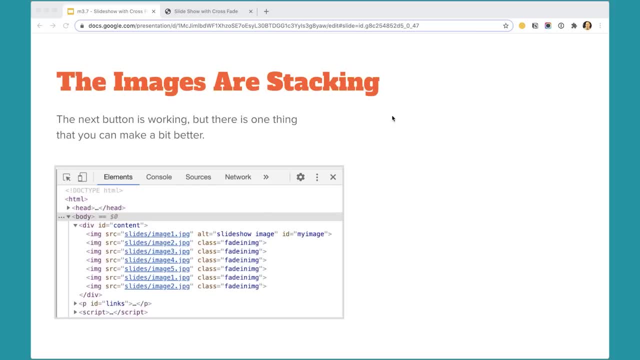 especially when it starts adding the same images to the dom over and over and over again. i think that it could be a little bit more efficient and a little bit better and a little bit cleaner. so what we're going to do is we're going to remove the extra. 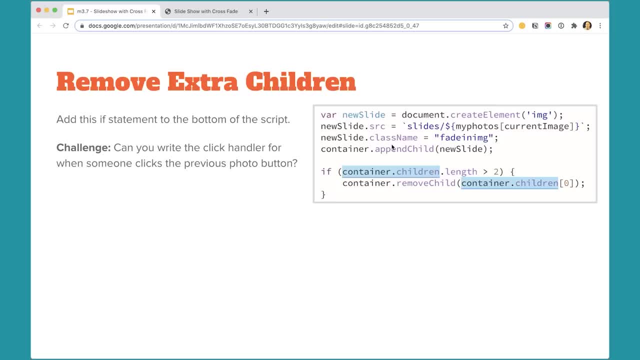 ones, the extra images, as the new images come in. so what we'll do is we'll say: okay, container, you have children. the children of the container are the images and if i'm gonna, if i have more than two images, if children dot length is greater than two. 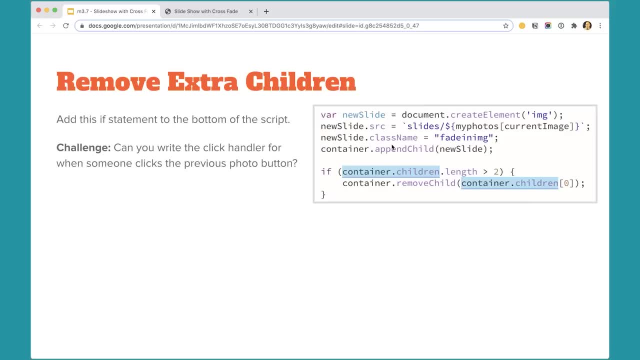 i'm going to remove the first one in that container, the bottom image. i'm going to remove the one from the very bottom of that list which is not showing anyway. it's it's at the bottom of the stack and it's not going to be seen anyway. so that means you'll have 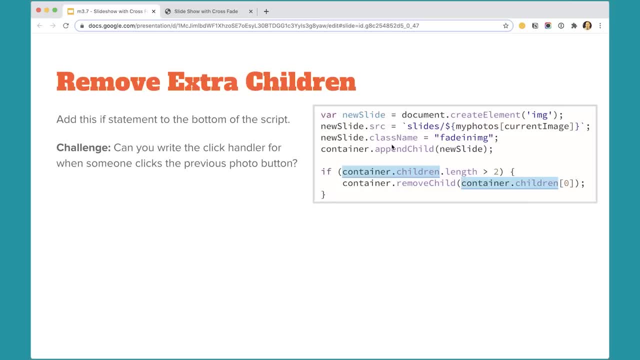 one image and then you'll put another image on top, and as soon as you click next and add a third image, then the one at the very bottom of the list will go away. so you never have more than two in the list, and i think that that makes the script a little bit. 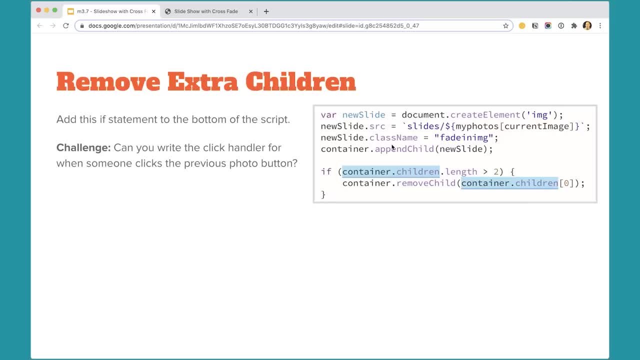 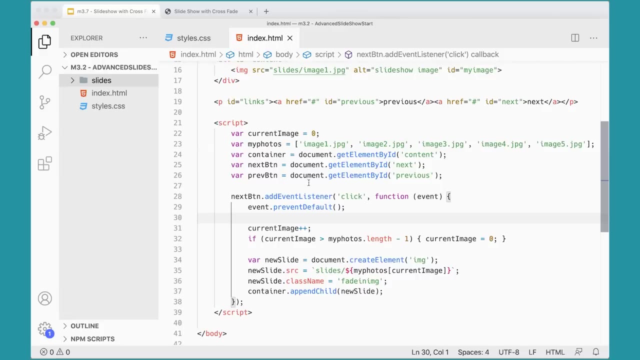 better a little bit, keeps our dom a little bit cleaner, because we're not continuing to add more and more elements every time somebody clicks the link for next. so let's go ahead and add this to our um, to our script over here. so down here i'm going to say: if 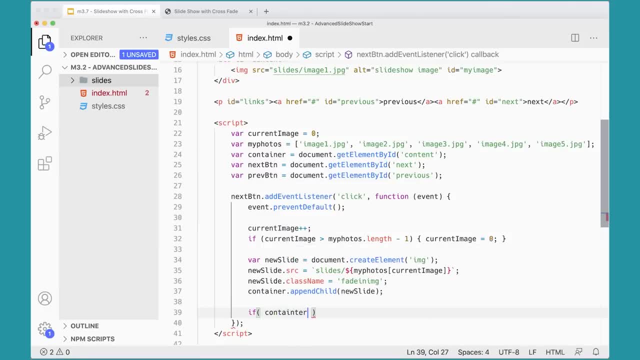 and in here i'm going to just put container dot, children dot length. if that's greater than two, then i want to do something. and what do i want to do if it's greater than two? what i want to do is i want to say container dot. 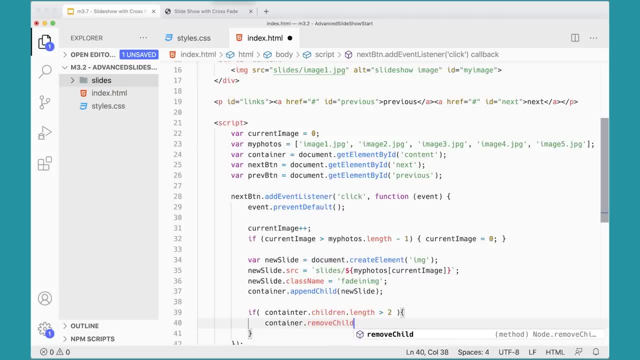 remove child. i want to remove a child. which child do i want to remove? i want to do container dot children. that'll be all of them. but i want to get square bracket zero. that will remove the bottom most child from the list and we're using the remove child. 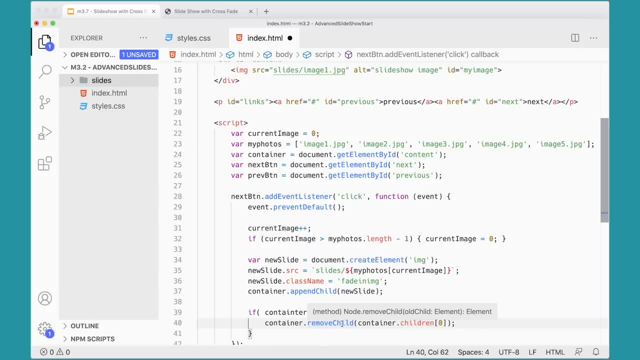 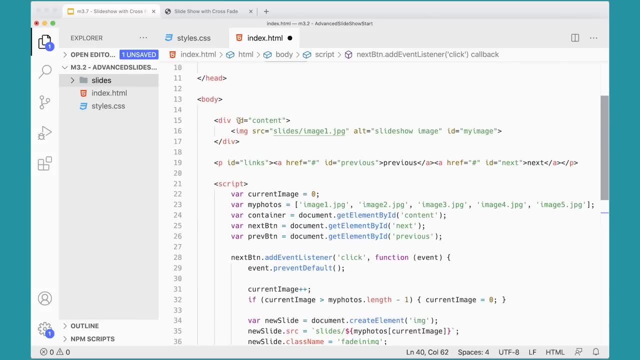 method, which is a document method that allows us to go into the document and remove a child from the, from a particular element, in this case the container. and again up here, the container is this thing, this dip, and it has children which are images. and this, when we start off the page, there's just 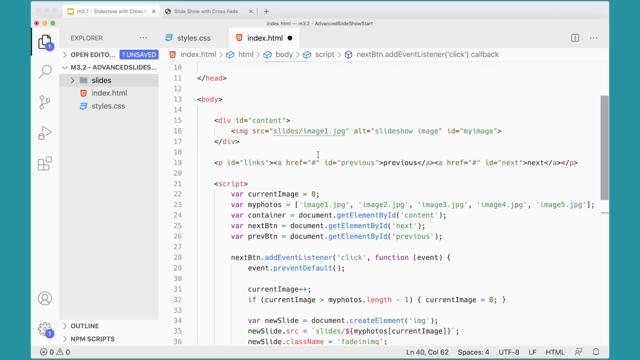 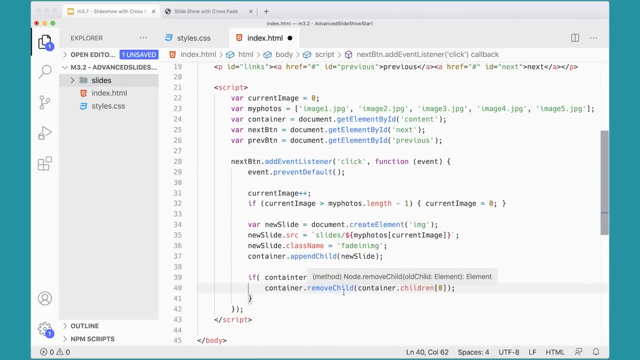 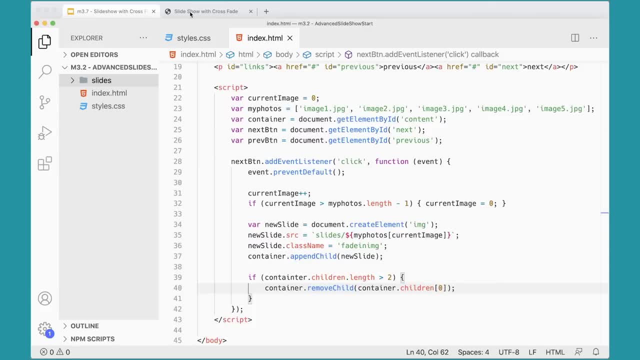 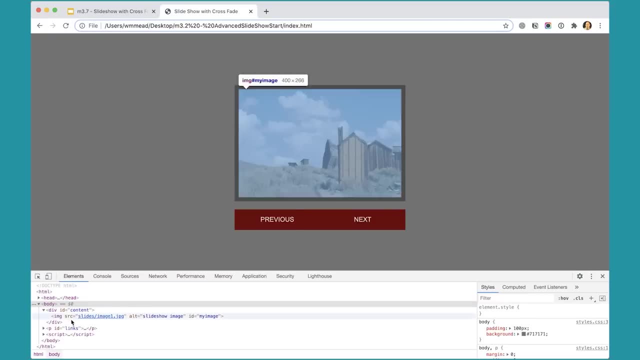 list. let's save this and see if i typed it all right and test it over here, and i'm going to look at my content here. you can see i've got one image there. i add one, so that adds image number two on there. and then now, if i 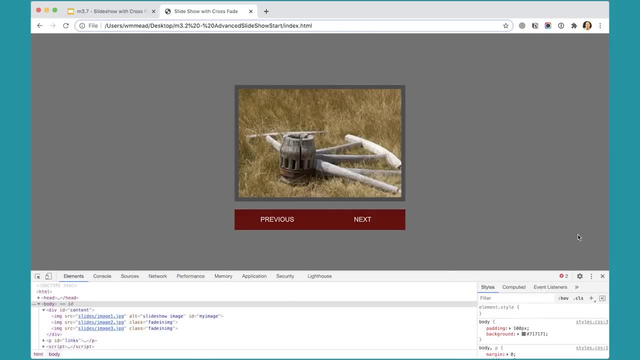 click it again. whoops. image number three: what did i do wrong over here? and this happens, you'll notice. over here i've got errors. so what did i do wrong? let's go to the console and see: oh, container is not defined. so this is a perfect example of a 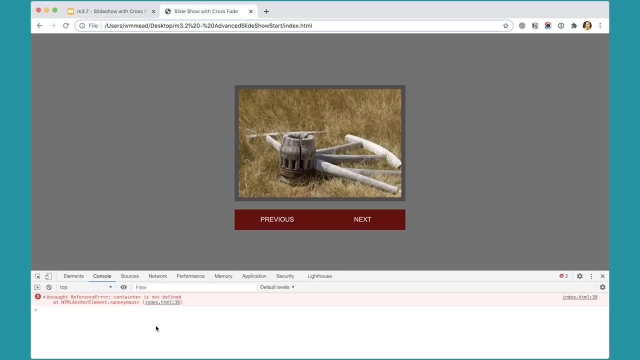 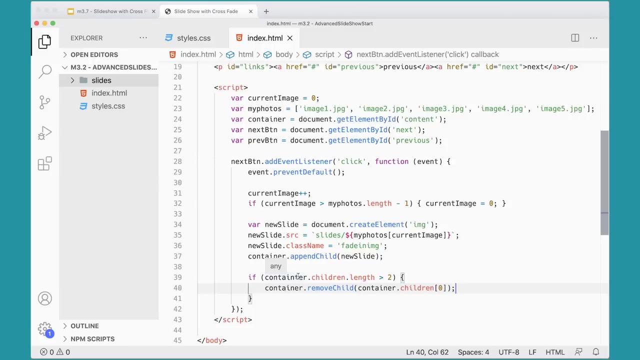 type of error that might come up will probably come up if you spell something wrong and it says over here: on line 39, container, line 39 container. line 39 container, container, container, container. there we go, let's try that. come back here. we all make misspellings, we all make mistakes, don't. 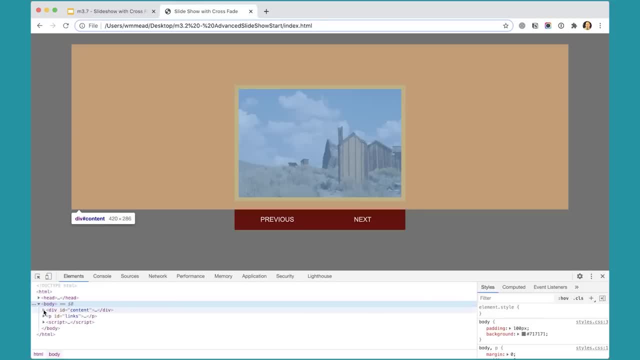 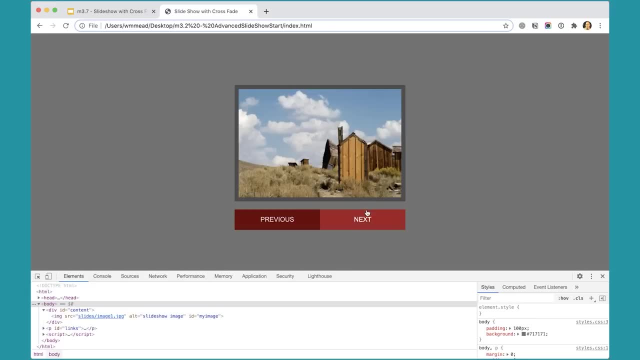 expect to not make mistakes. it's great when those come up while i'm doing this, because then you get to see how i fix it all right. so coming in here i can click next and it's adding that on there. you'll notice i'm not getting the error now. 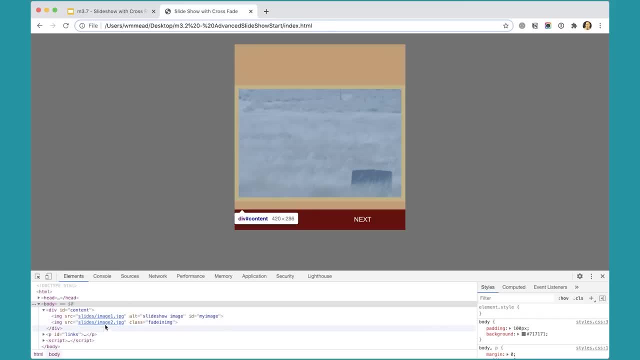 and now, when i click the third one, it should add the third image but also remove the first one at the bottom there, or really at the top of this list, but really this one is underneath that one, so that's what i mean by bottom. so now we've. 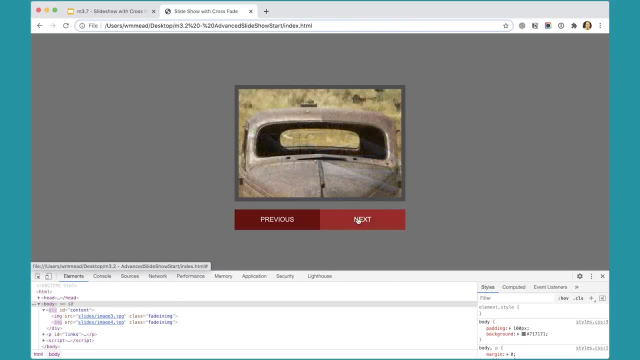 added image 3, but image 1 went away and i can keep going and i'll do image 4 on top of there and then image 5. we've got 4 and 5 on the screen. 4 is on the bottom, 5 is on the top. 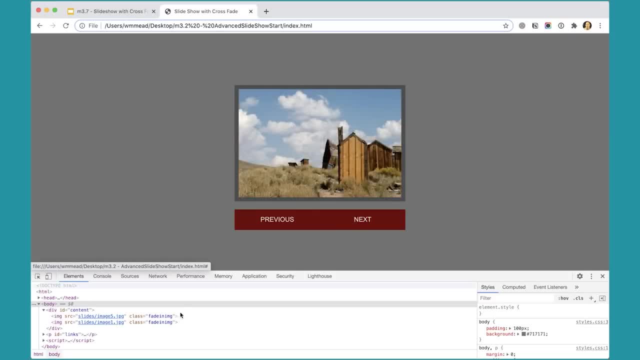 and image 1 is now on the top. you might be wondering why the one down here at the bottom is on the top. you have to remember the page renders from the top to the bottom and the fact that these are set to position absolute means that this one. 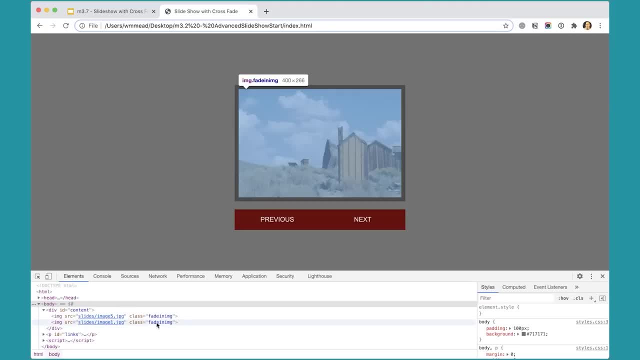 gets added to the page first and then this one gets added to the page second, and because it gets added to the page second, and because of the absolute positioning, that means it ends up on top- it's on top of the first image, so that's working just great. 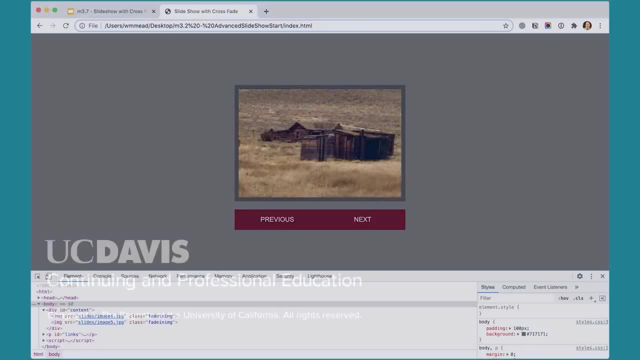 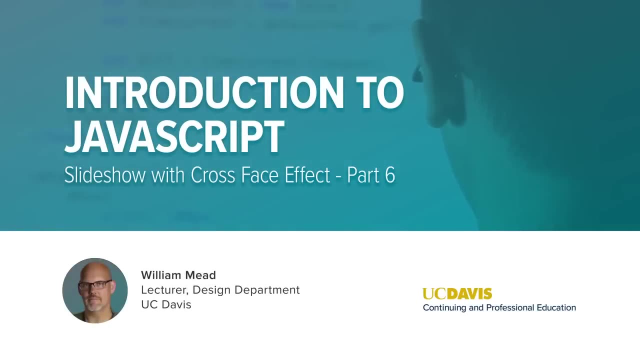 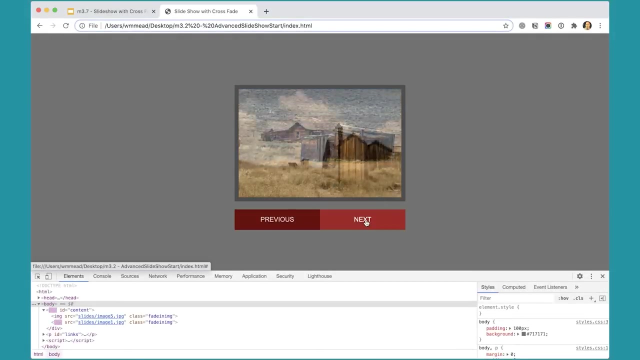 exactly what we want. we have our next button working just fine, so i can click next and it will go through the slides. and not only that, but it's kind of nice and clean because it removes any extra slides we don't need, as it's adding new slides. 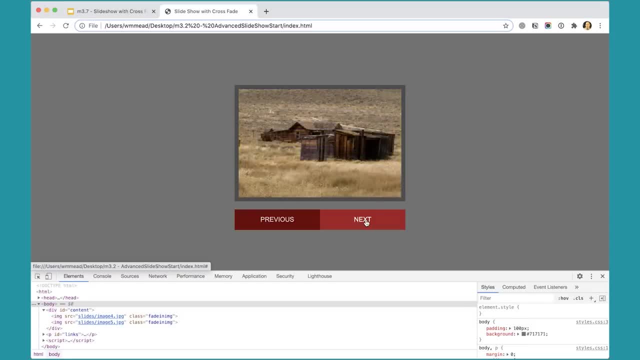 on top. so that's really neat and that's working. so now the question is: how do we get the previous button to work, because currently clicking that does nothing but reset the page and notice we're getting the hashtag up here. so how do we get the previous button to work? 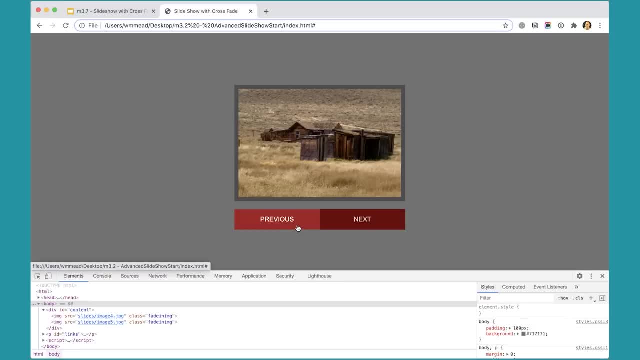 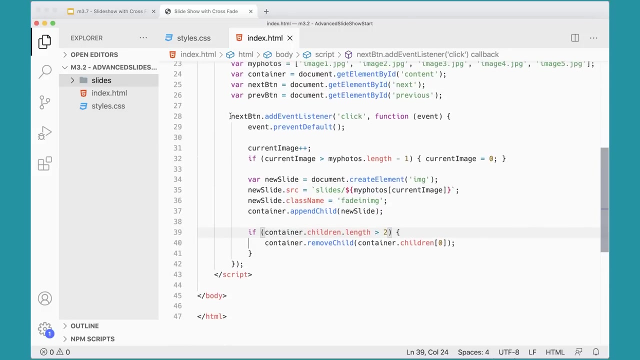 what we want to do is pretty much the same thing that we did with the next button, but with the previous button, and see if you can do that challenge on your own, and you can even go ahead and take this function that we've written for the next button here. 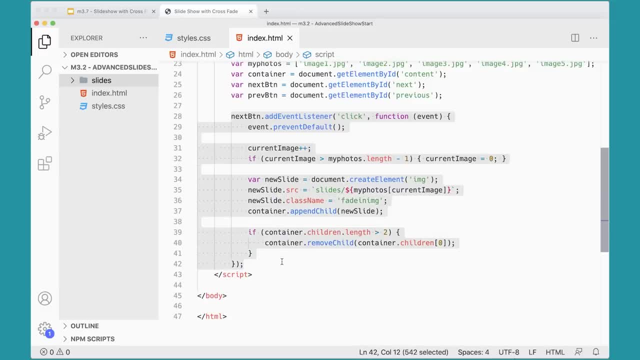 this one here, copy and paste it and see what you need to change to make it work for the previous button and, just like before, you can use- you can actually use- the previous slideshow, the previous project, the earlier version of the slideshow, to figure out how to do this. 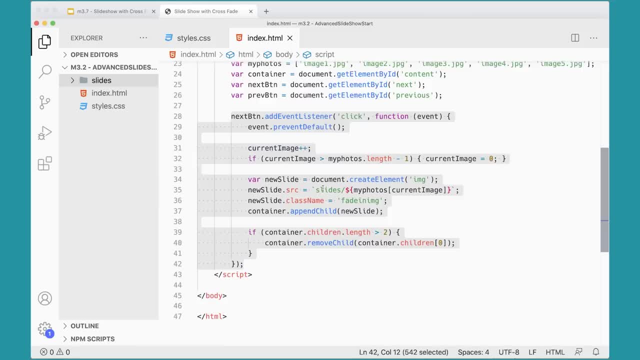 because we're going to decrement the image and this is going to change, but all of this is going to remain exactly the same. so see if you can do it on your own. pause this video and come back when you've tried it, and either you've gotten it to work or you haven't gotten it to work. 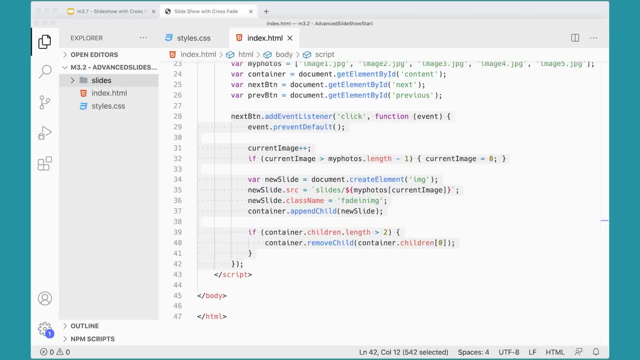 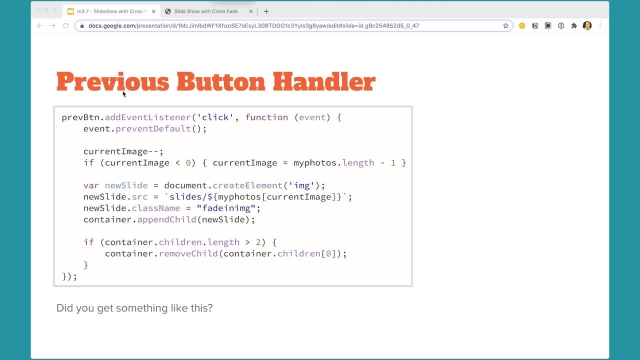 now. even if you don't get it to work, that's okay. try to do it on your own. did you get something like this? hopefully you did. let's take a look at what's changed here. what's changed is here. we're putting the event listener on the previous button. 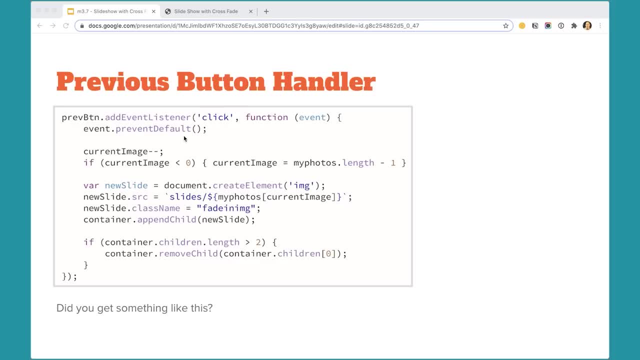 instead of the next button, so that's different. the rest of this is all the same. instead of incrementing current image, we're decrementing it, so that's different. and then down here, the if statement has changed a little bit. if the current image is less than zero, we're. 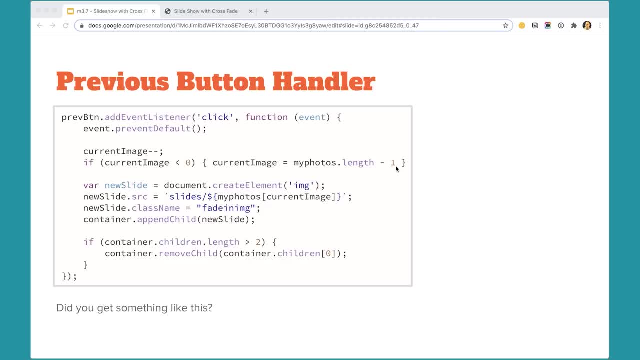 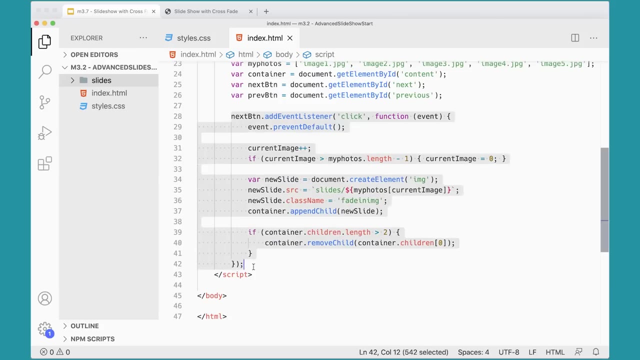 setting current image to photos length minus one, just like we did in the previous slideshow. so other than that, everything else is the same, so let's see if we can actually make this work over here. I'm going to copy this script and then paste it here and just change this to: 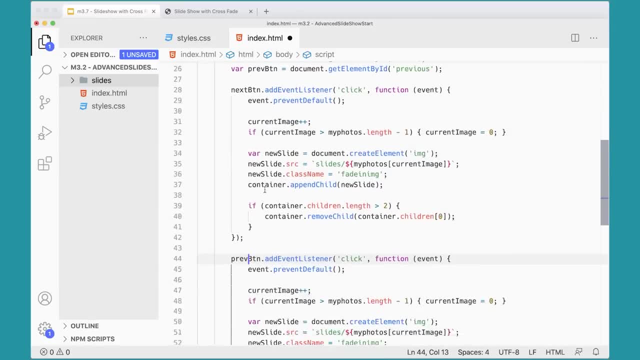 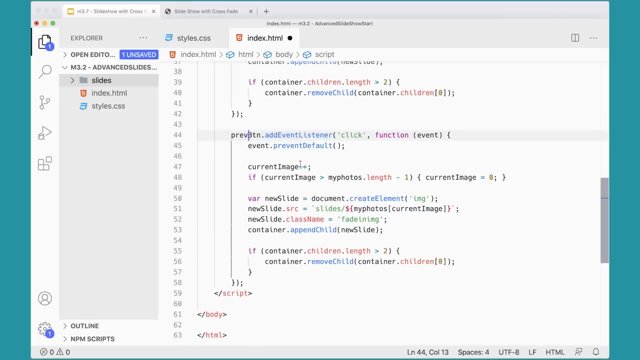 prevbtn, which is what I have up here: prevbtn. so that's going to go into the dom and get that button and add the event listener to it, and all this stuff is the same. the only thing that's different is here this gets decremented and then down here. 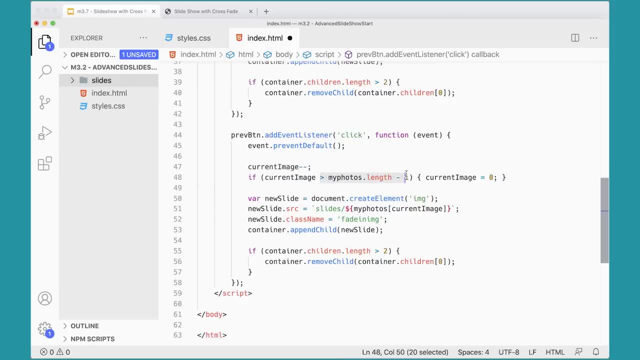 if this is less than zero, then we're going to set current image to my photos, length minus one. okay, so that's going to set that all up there to work for the current image for that one, and that should be it. that's all we need, the rest. 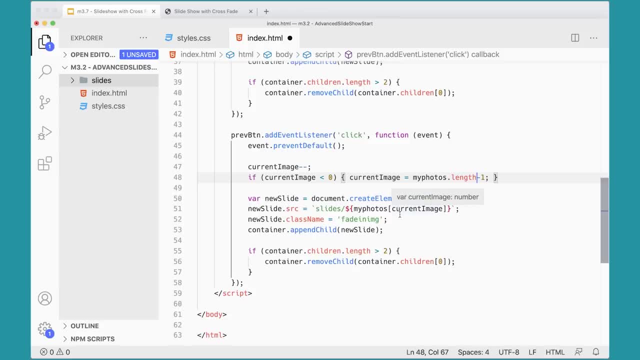 is going to be the same. we're still going to create an image, we're still going to go get the get the image from the array based on the value of current image here, and then we're still going to apply that class to it and we're. 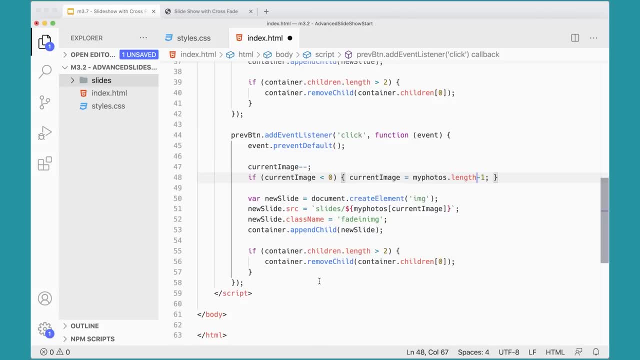 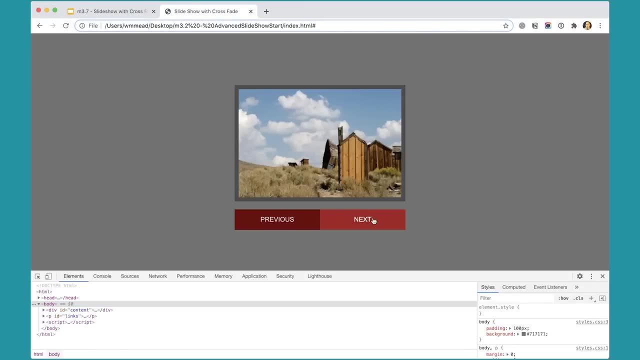 going to still put it on the page and we're still going to remove the extra children, so all the rest should be the same. let's see if this works. come back and click refresh next works. I can add images and over here you can see they're getting. 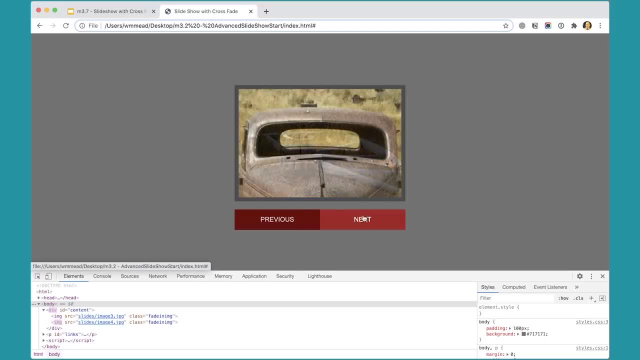 added image two, image three, I could add one more, image four, and now when I click previous, you can see image three got put on top and image four is now on the bottom. image two is now on top. image three is on the bottom, image one and then. 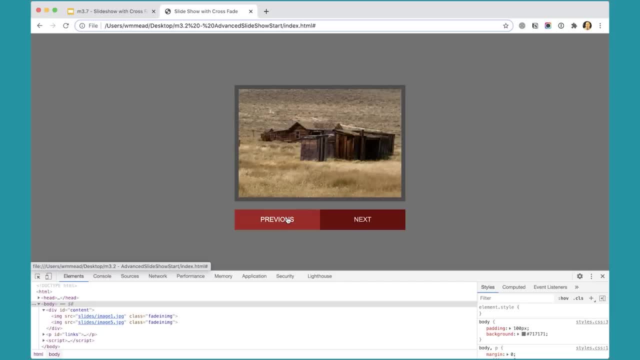 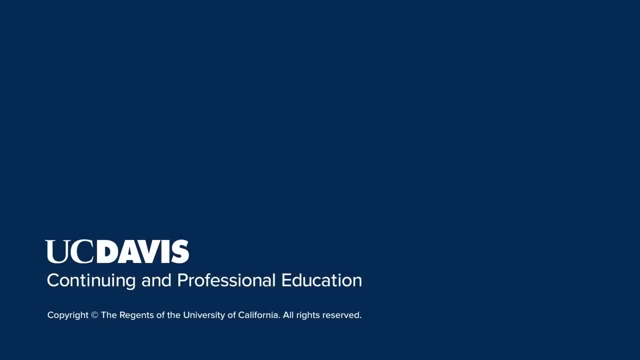 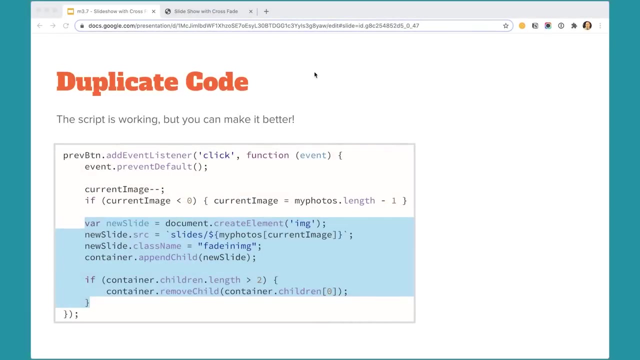 image five, because we're going to the end of the array and then back on down through the array, like that. so that's working perfectly, just exactly what we want. your script is working great and you could just leave it the way it is. it's totally fine. 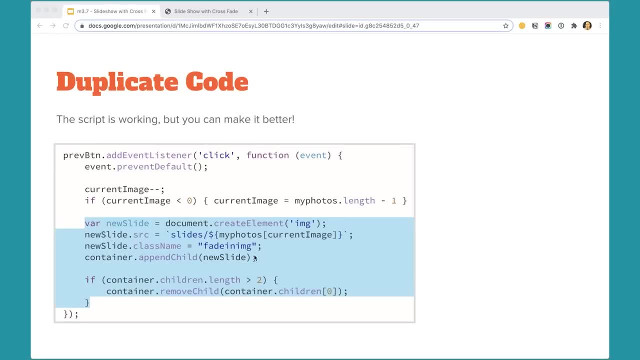 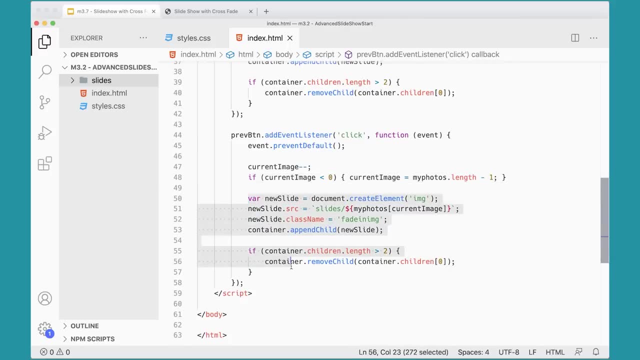 but you'll notice that we have a fair amount of duplicate code if we go over and look at our script. we've got this chunk of code in here. that's a good. you know several lines of code which is exactly the same as this chunk of code. 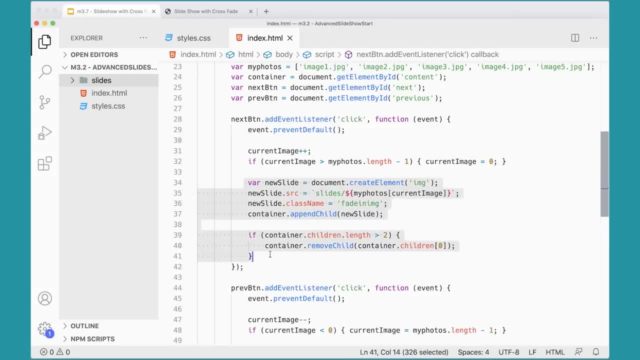 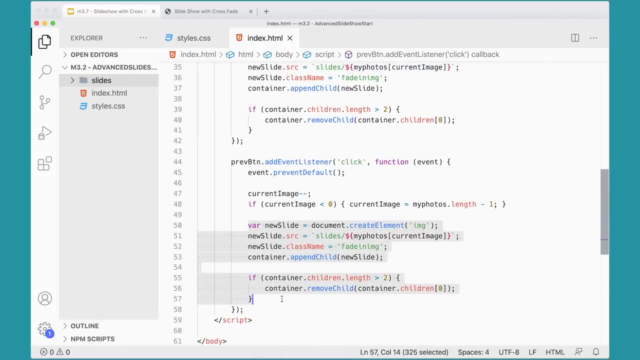 up here and there's a concept in programming called don't repeat yourself. dry don't repeat yourself. so what we want to do is, instead of repeat this code twice, pull it out and put it into a separate function. we're going to make a function called swap image. 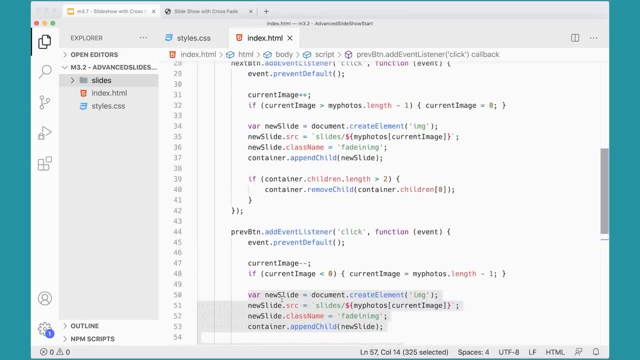 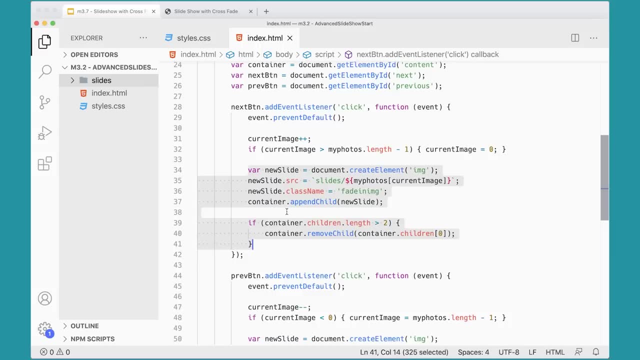 something like that, and that function is going to have this chunk of code in it and then, instead of having this chunk of code here in each of these event listeners, we can just run that function twice: once in the next button event listener function and one in the previous event. 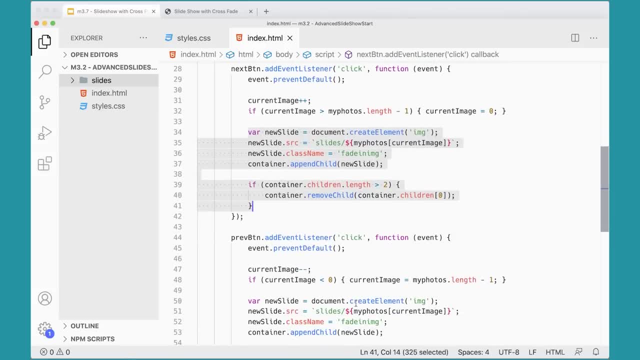 listener button function. so try to do that on your own. see if you can pull that code out, put it in a separate function and give that function a name and then call that function here inside these functions and see if you can do that on your own. pause this. 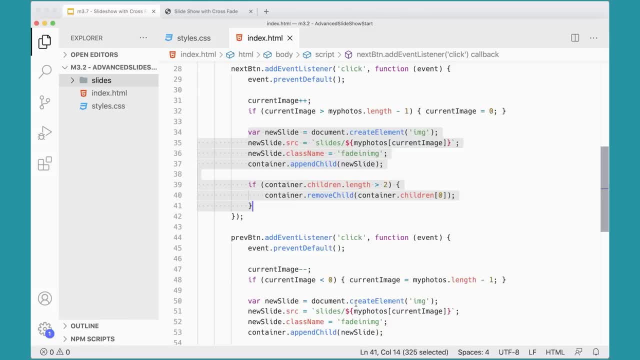 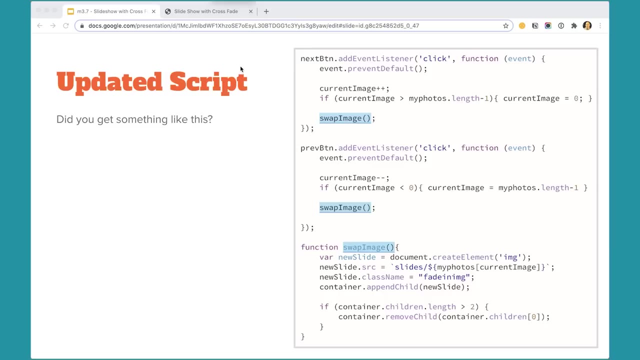 video now and try it, and if you can't figure it out, or once you do figure it out, continue with the video to see if you got the same thing that i got. did you get something like this? i hope you did. you may have named it something. 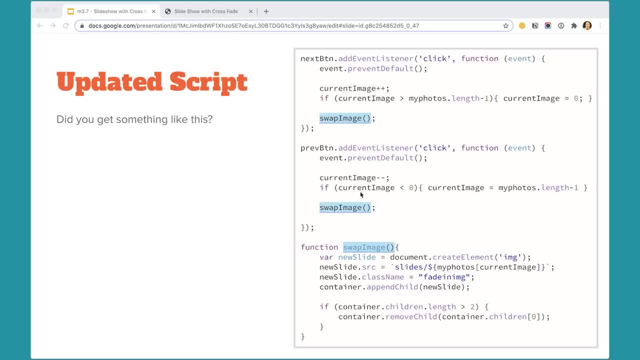 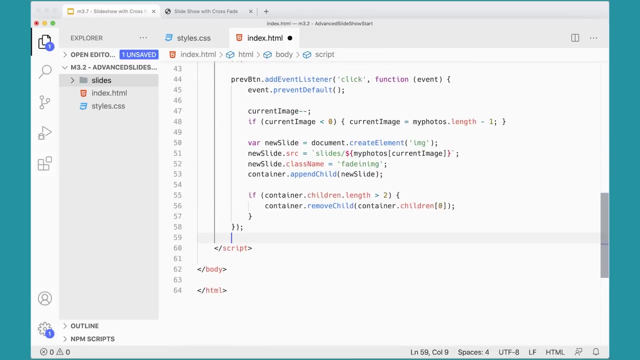 slightly different, and that's fine, but this is what i named it: swap image. and down here i have a swap image function. let's do this together, just in case you got stuck and, um, you can see how i would go about doing this. so down here i'm going to make a new function. 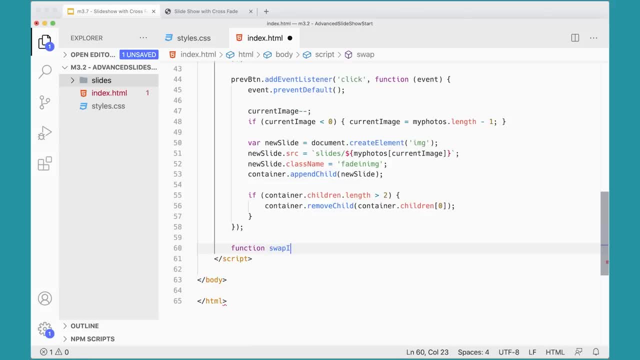 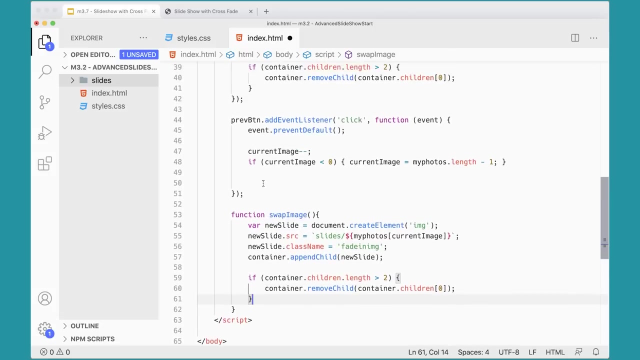 function, swap image, and then that function is going to contain all of this stuff in here, so i can cut that and stick it inside this function. there we go, and now, instead of having that up there, i can just run swap image right here. i can also run it. 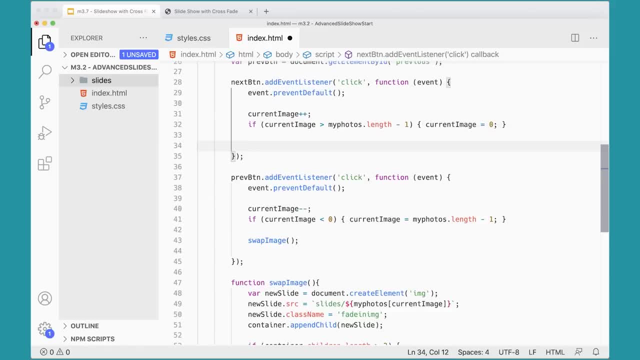 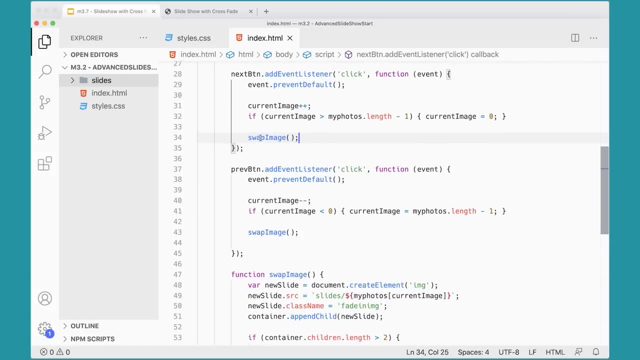 here in place of this stuff, because it's all exactly the same. there we go. so now we've got a function called swap image that will run twice. it'll run the same function, basically if you're clicking the next button or the previous button, and that kind of cleans up our code. 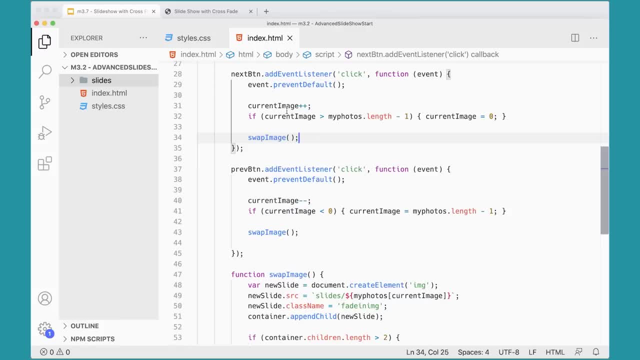 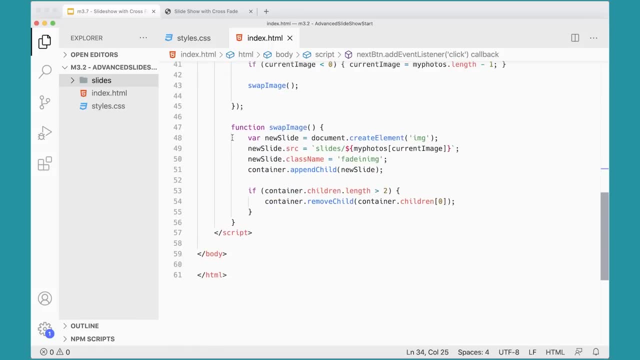 because we can see here very clearly that the next button is incrementing this variable and and then checking with an if statement and then running function, and we can come down here and we can see what that function does very easily without any fuss or muss. so that kind of really cleans. 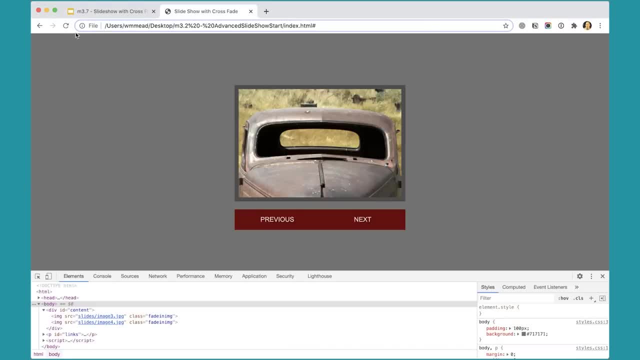 up the code a bit. let's test it and make sure we did it right. so over here i'm going to refresh the page. if i click next, you can see that the script is working exactly the same as it did before. nothing else is changed. really, we're not adding any new functionality. 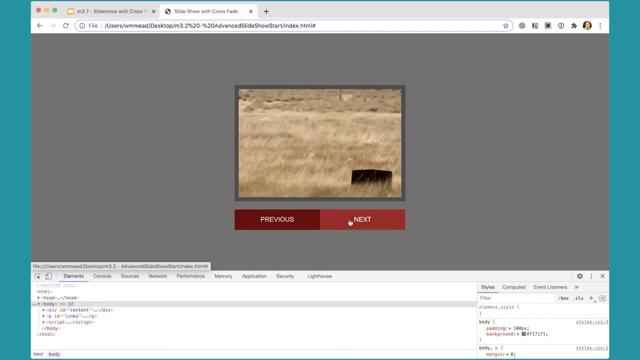 we're just refactoring our code. you always want to refactor your code and try to make it better, and try to reduce the amount of code or make it cleaner or make it easier to read- all of these things you want to do, and often, when you're working on projects, you'll find: 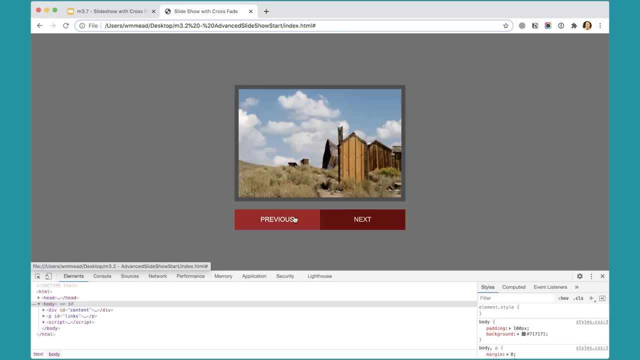 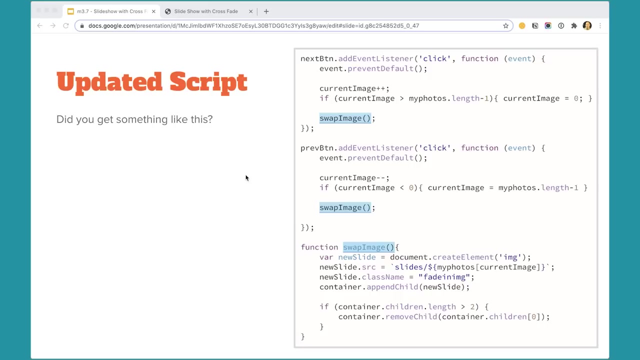 ways. you'll look at an old piece of code and you go, oh wow, i could have made that simpler. and you'll do that, and that's just part of the normal process for any programmer. now the very last thing to do here is to put it in a separate linked file. 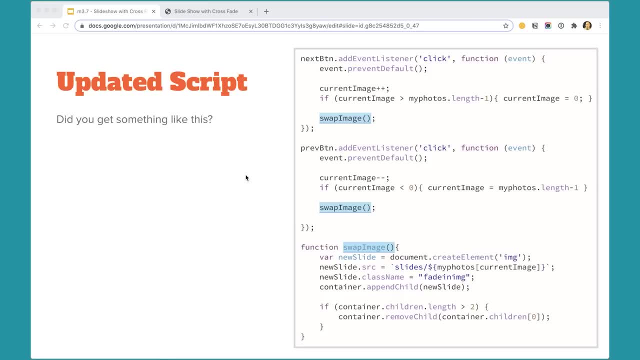 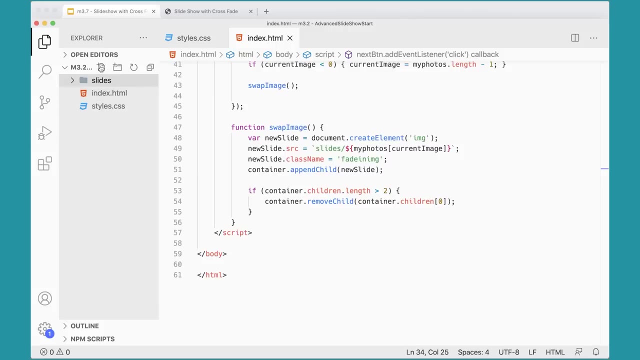 and to do all of our nice clean up stuff, to follow best practices for, for scope and for everything else. so let's do that quickly together as well. so i'm going to come back to my file over here. i'm going to make a new file on here. click new file here. 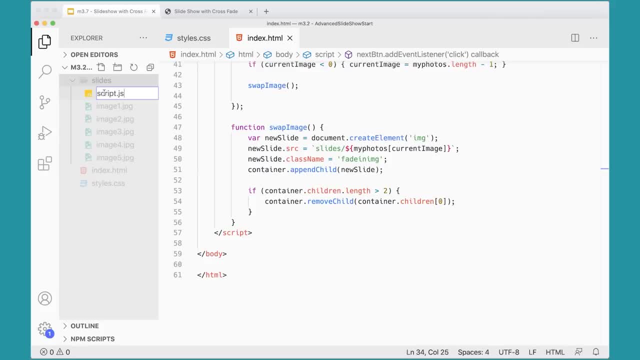 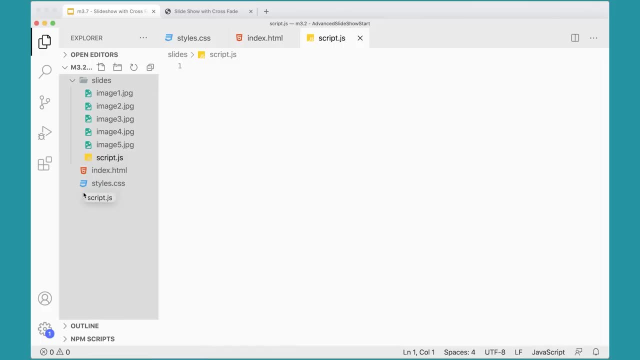 and call it script dot js. and look at that. i've made a mistake, because i can see it's putting it inside my slides folder, which is not where i want it, so i'm going to actually move that out here. are you sure you want to move? yes, 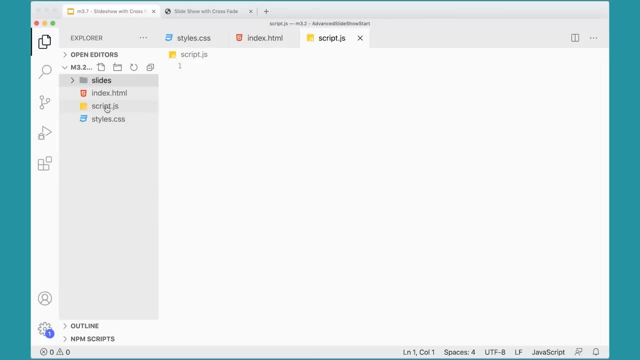 move. so now it's here. so make sure it's not inside the slides folder. it's here scriptjs, and you could put it inside the slides folder and link it there. it just doesn't really make a lot of logical sense to put it in there, okay, so? 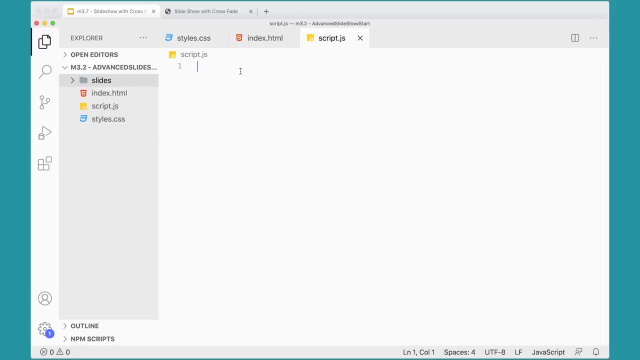 on the script file. once again, i'm going to add my immediately invoked function function parentheses, curly braces and then an additional set of parentheses and a semicolon. it's terrible syntax, but that's what we do here. this function will run immediately when the page runs and then click between the curly 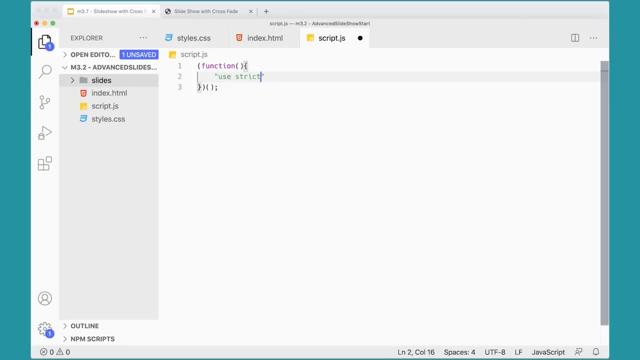 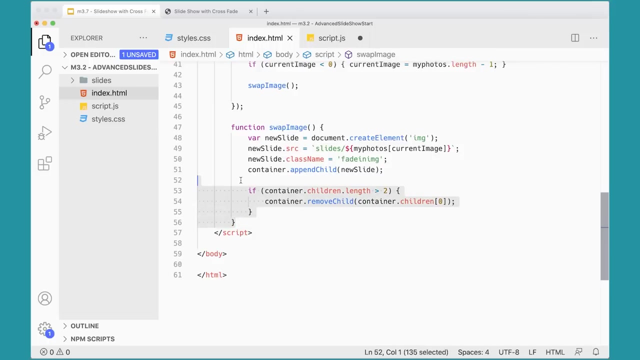 braces and move that down, and we're going to add use strict in here. so that's great. so we've got you stripped in there and now we can come over here to our to grab our script from here. we're just going to grab everything inside our script tags, all the 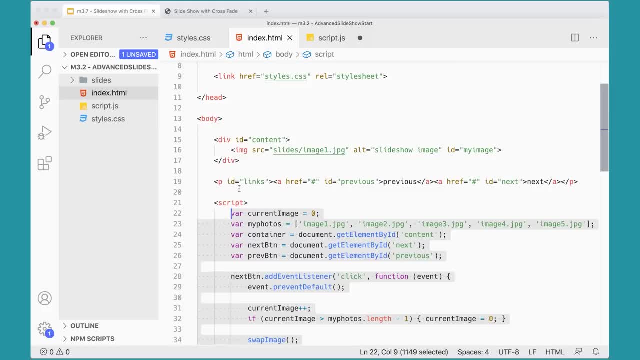 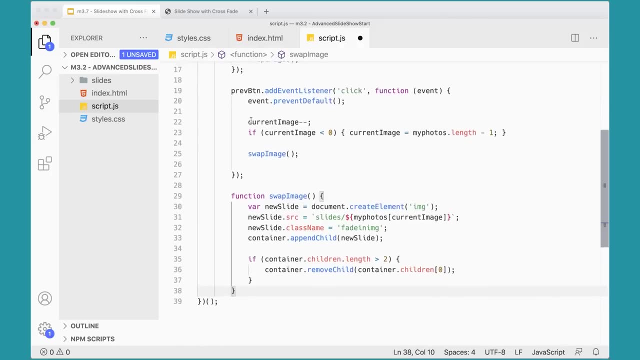 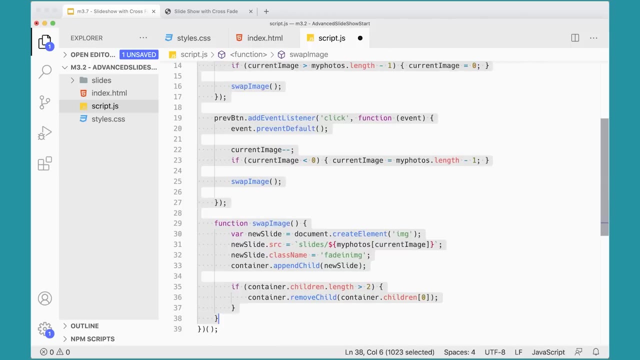 way up to the very top of the script tag here. i'm going to copy that and i'm going to stick it over here and paste it in there and i'm going to actually shift tab to move it back. so now that's in there. that's good. now the last thing i want to do. 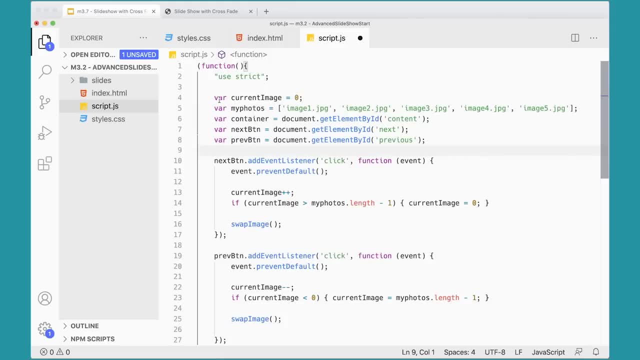 is. i want to go through and fix the variables here. this one current image is going to change, that variable is going to change down here we can see that. so that needs to be let. but the rest of these can all be const, const, const, const, because those aren't going to change during. 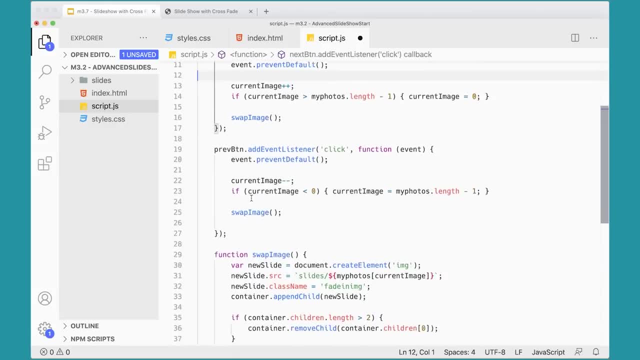 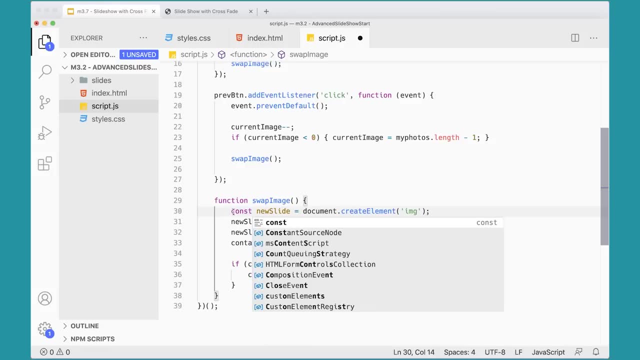 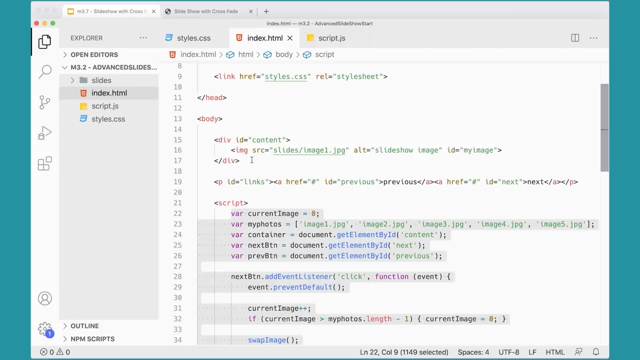 the script at all during the running of the script and then down in the swap image. we have a variable here that one can also be const- great. so we've got that. so now we've got our file all set and that's all looking good over here on our 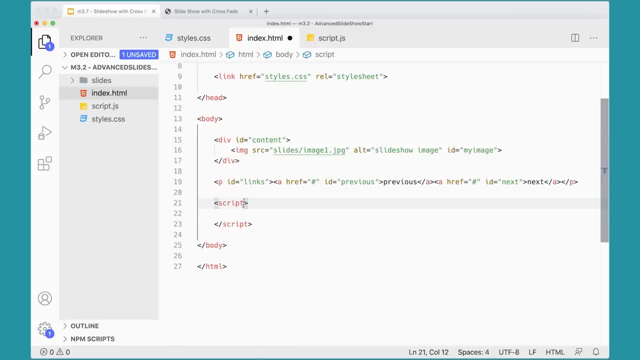 index file. we just need to get rid of that stuff and put in here src equals. src equals scriptjs. that's our file and we can put this up here like. so we could leave it like that or, even better, we could take this and move it up here into. 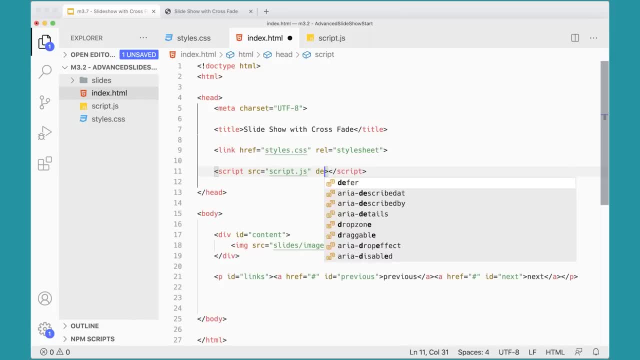 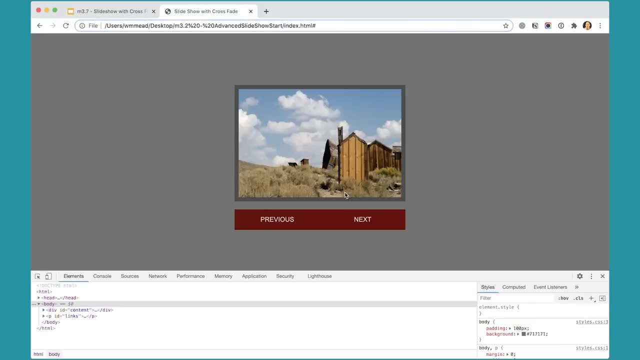 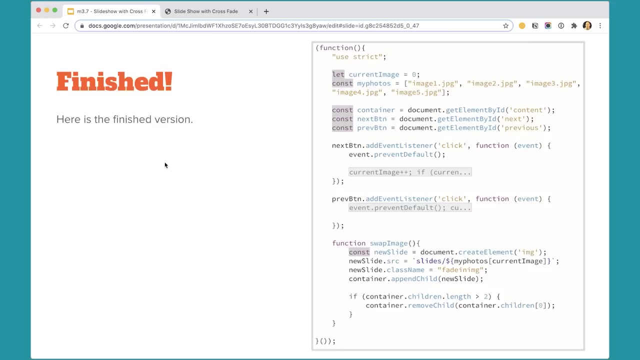 the head of the page and add the defer attribute here. save that and then always check to make sure you didn't mess things up along the way. and look at that, it's working perfectly. everything works great. so there we go. we have finished our script and we've cleaned it all up. 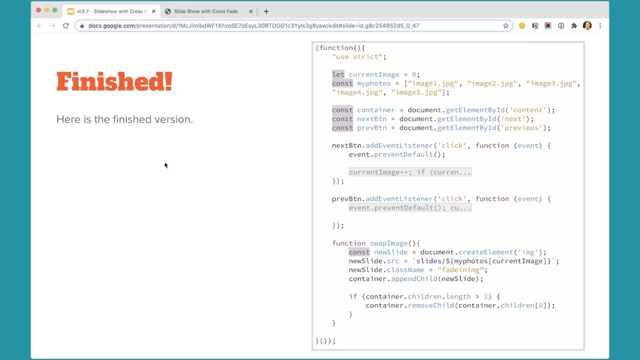 and in this lesson you've learned a lot about some different ways of doing things and how to add elements to the page and remove them from the page, all with using our document object model as well as our event handlers, and this is a really great little slideshow that you could use on. 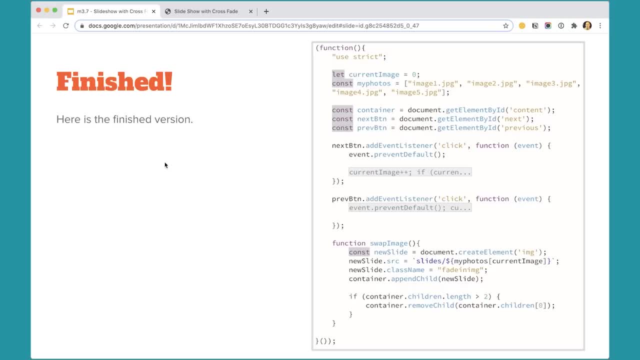 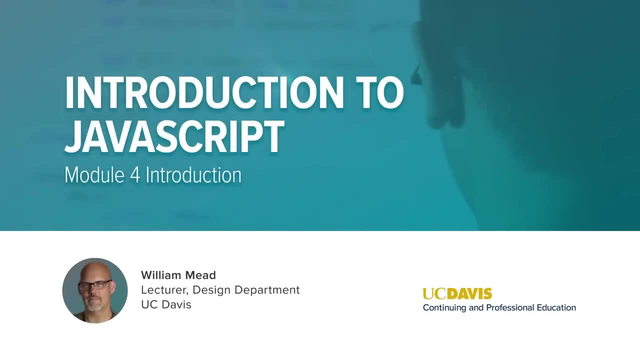 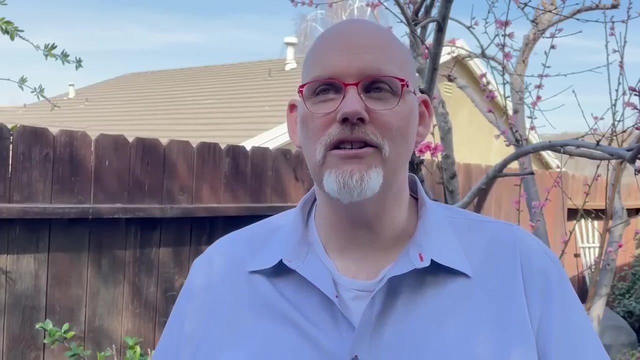 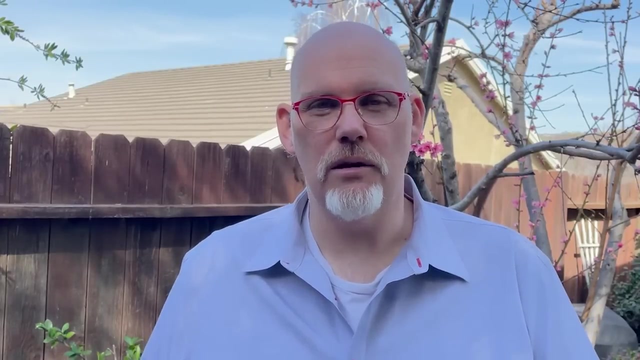 any webpage and, yeah, I think this is a great, great project. hello and welcome to the fourth module of this course. congratulations for making it this far. you've learned a lot of javascript so far and this fourth module is going to really help you push your skills even further in this module. 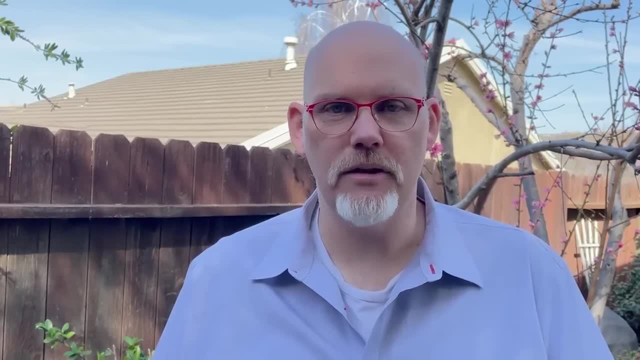 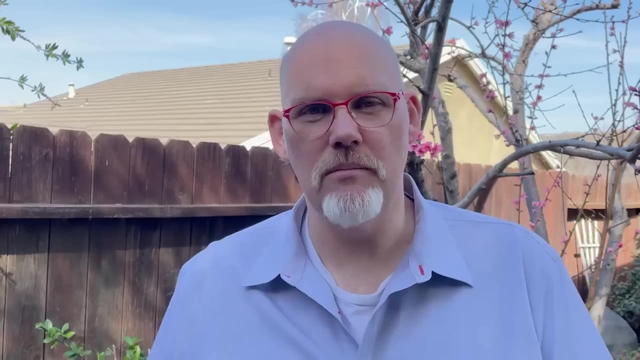 we'll be doing a lot of practice. to learn javascript, you really have to practice. you have to get used to the syntax. you have to think about how to break problems down into smaller pieces to actually make something that works, and we'll be doing that in this. 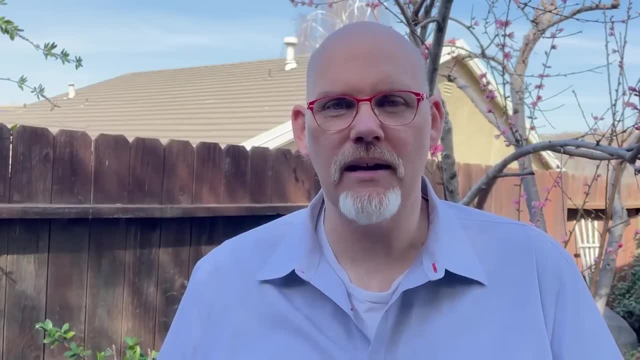 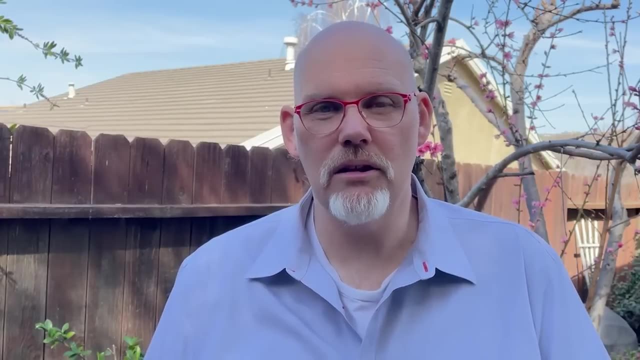 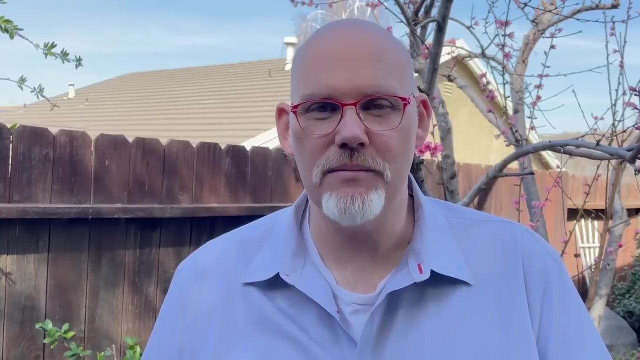 fourth module, and by creating interactive elements and practicing what you've already learned, you'll be making some things that are interesting and fun, but also really learning javascript along the way. so let's get to it and hopefully by the end of this module you'll be really excited about what you've learned. 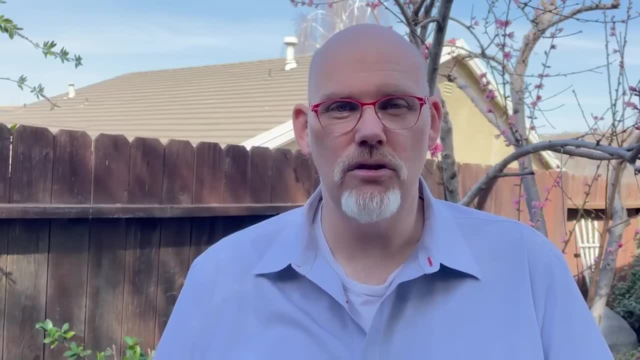 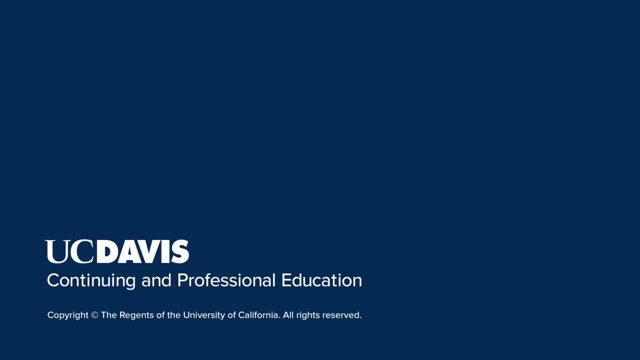 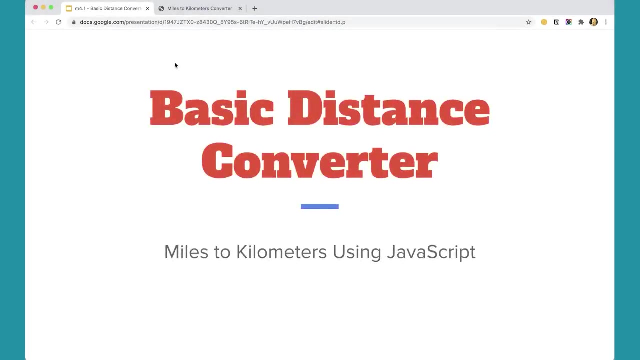 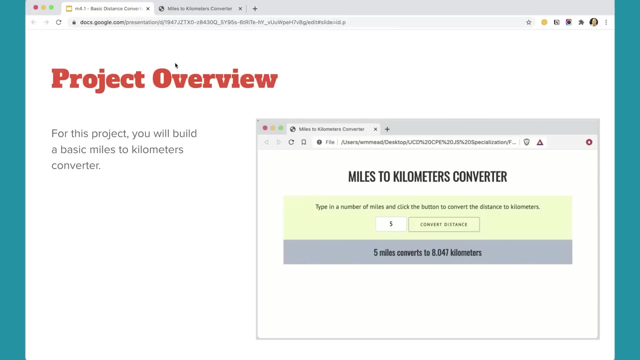 so far in this course and you'll be excited to go on to the next course and learn even more about javascript. in this project, we'll take an interface that I've already created and make it work, so that we end up with this little tool that will convert. 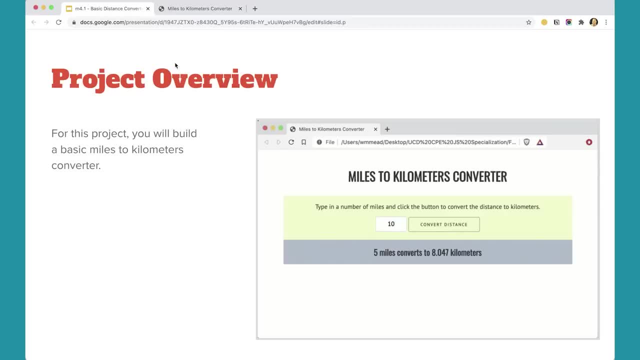 miles to kilometers, and through doing this project you'll get to use a bunch of the pieces we've talked about already: learning javascript, you'll capture data from a form element and manipulate the dom, change the dom by adding this actual conversion down here, and we'll do a bunch of the different types. 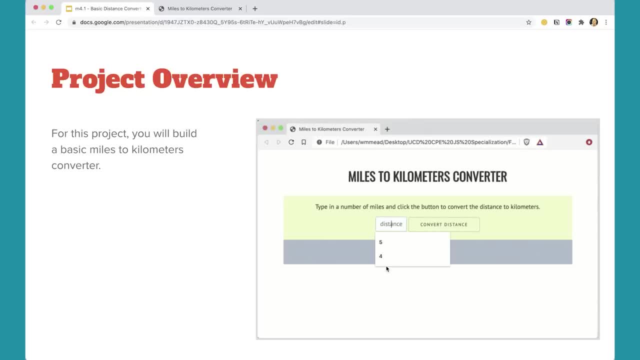 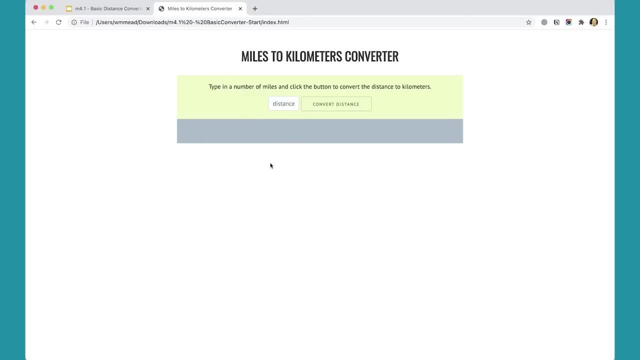 of things that we've been doing so far with javascript to create this little tool, and the interface is already created. you can see I have it over here. the html generates this interface, but at this point it doesn't function. so our job today is to make this thing actually function and write. 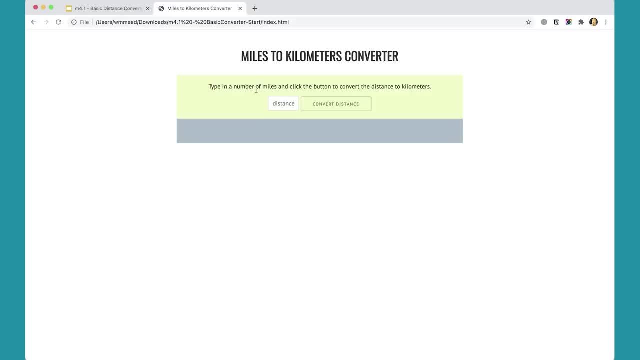 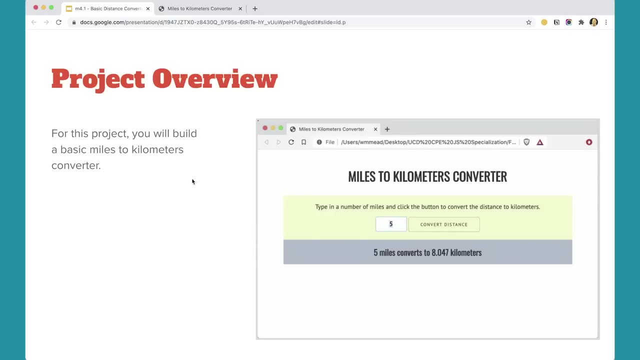 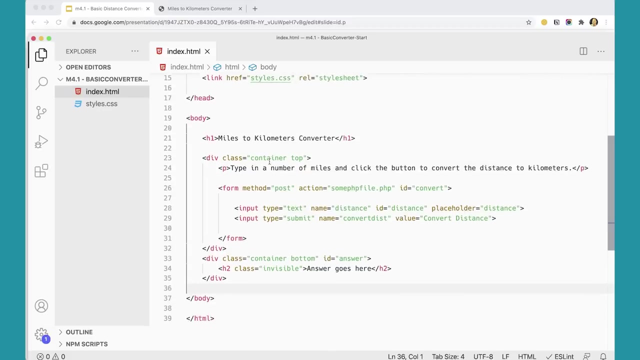 the javascript to take the data that somebody types into distance and convert it to miles, so I mean convert it to kilometers. so yeah, let's take a quick look at the html that we have here. nothing too fancy here, we just have some basic html with a form. 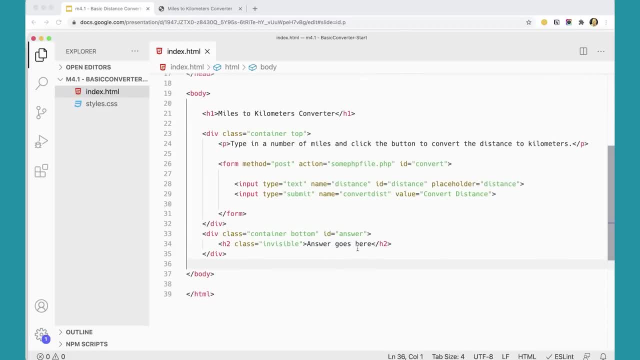 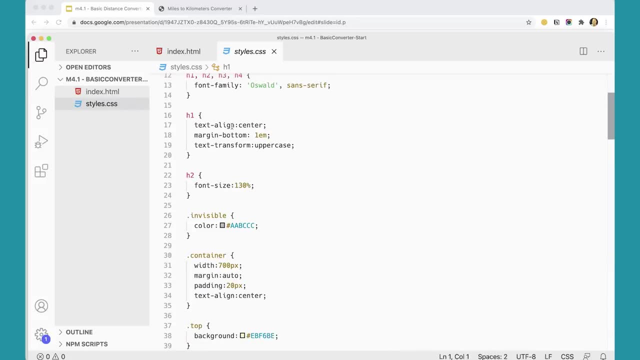 and a container down here where the answer is going to go when we convert the miles. and then I've got some styling over here already in place, probably more styling than I really need, but that's ok, we don't need to touch any of that at this point. what we're going to do: 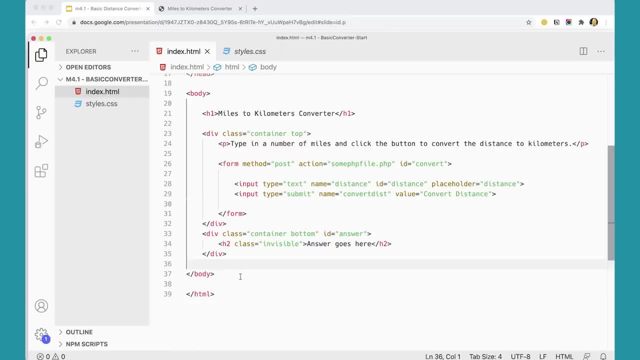 is, we're going to add a script tag down at the bottom and start figuring out how we're going to capture this. so let's do that. let's go ahead and add a script tag here and then, in here, we want to capture the submission of this form here. 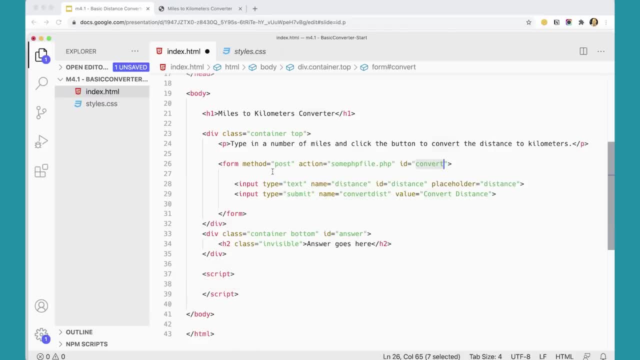 called convert. so we've got an id for the form, so convert. so we want to do down here, we want to have a document getElementById, getElementById- and then we want to get the id convert and we want to add an event listener- addEventListener. 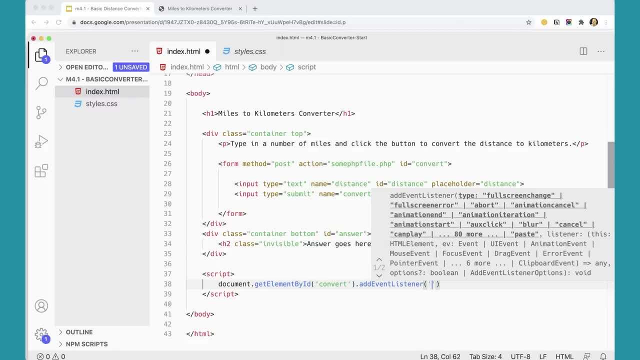 addEventListener, and the event we want to capture is a submit event when the form is submitted. we want to do something, and what do we want to do? we want to run a function. now. all the rest of the code for this script is going to go between these. 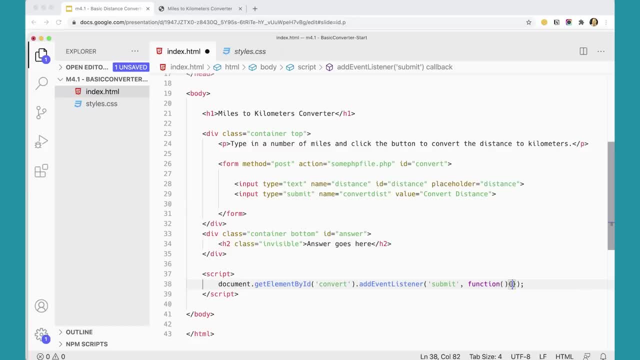 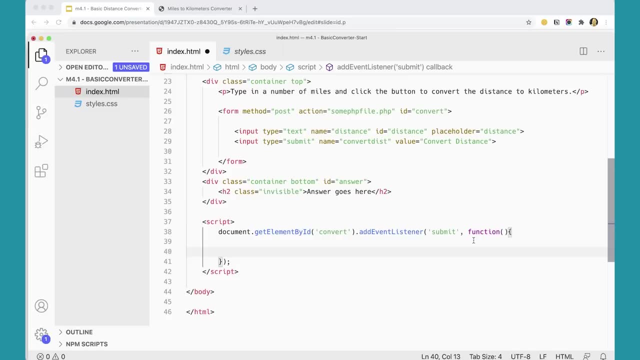 two curly braces here inside this anonymous function so I can click there and move that down. okay, great, so we've got our event listener here now. normally, when events happen like a submission of a form, what happens is either the data from the form goes to- if you have an action, 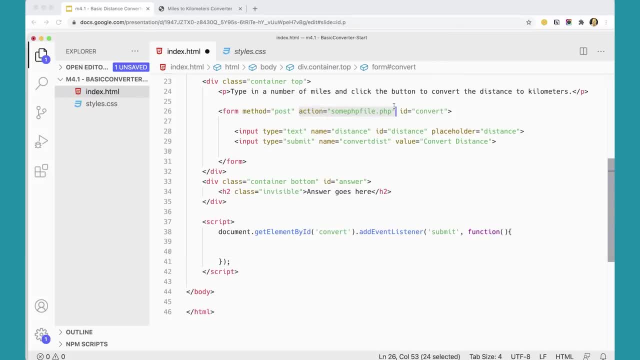 in here, like we do here on this form, it would go to some PHP file to be handled. or if you don't have an action, if you don't have this attribute here at all, then what it'll do is it'll actually refresh the web page, and we don't want that to happen. 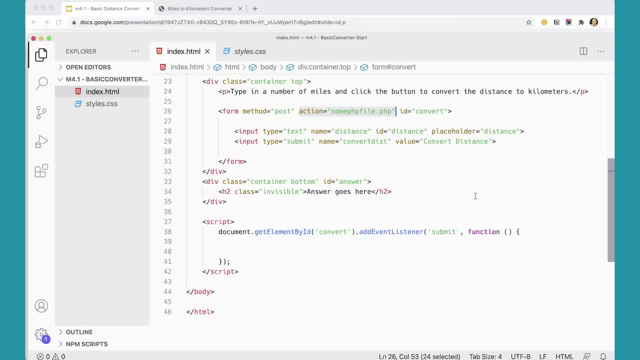 we want to stop the normal processing of the form, so in that case we're going to pass in the special event object and we could pass it in as event. or some people pass it in as evt, or some people just use e. I'm going to leave it as event, just to. 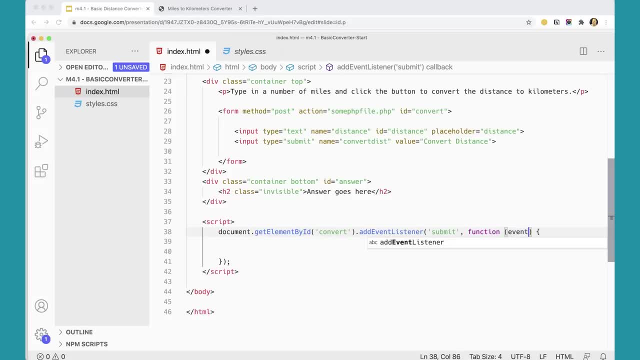 make it clear that that's what it is. it's the special event object, and then we're going to keep that form from being processed by using event dot prevent default, which is a method that will keep that form from getting processed and from refreshing the page, or 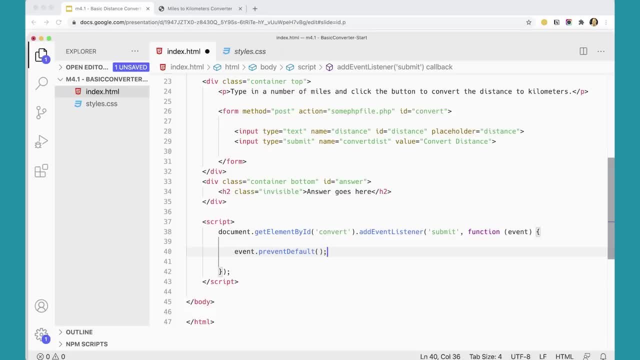 trying to go to that PHP file when we submit the form. so that's the thing we want to do first here. the next thing that we want to do is we want to capture the data that somebody typed into this input field here- the ID of distance. so we want to capture that data. 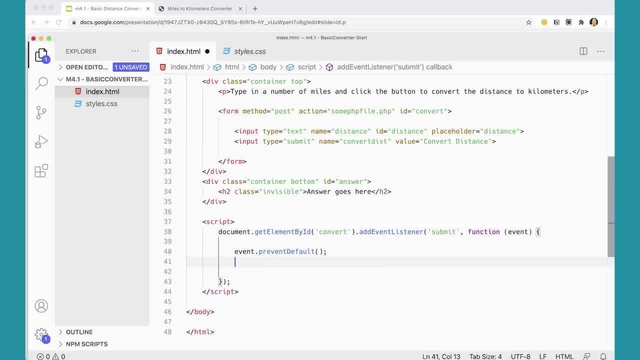 and we want to put it into a variable. so let's make a variable distance, var distance. and then how would we capture that data? do you remember how to get that data out of that field? see if you can think about how to type in the rest of this on your own. 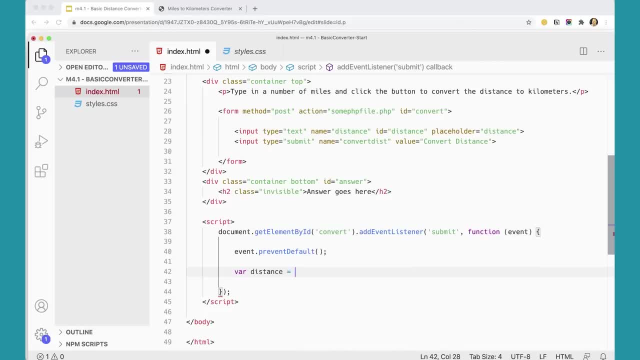 for a second and try it. try to see what you can get. see if you get what Matt and batches what I do here. okay, I'm going to go ahead and put mine in, but hopefully this is what you got. document dot. get element by ID and which ID? 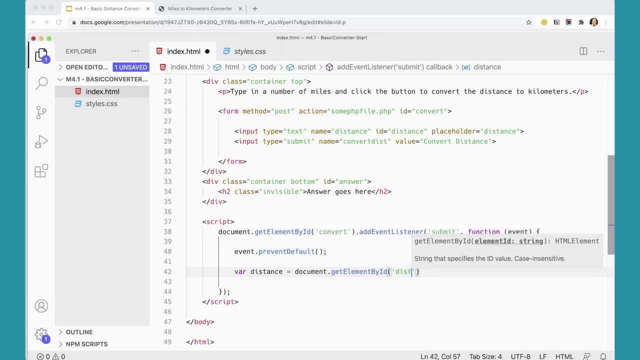 do I want? I want this ID distance, and what do I want from there? I want the dot value that's going to take whatever somebody has typed into the field and stick it into this variable distance. let's give it a try real quick. if we do alert. 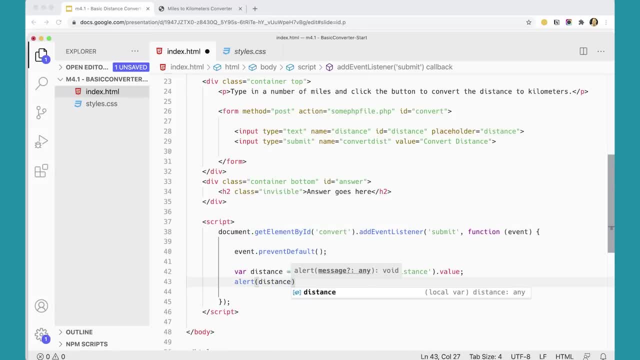 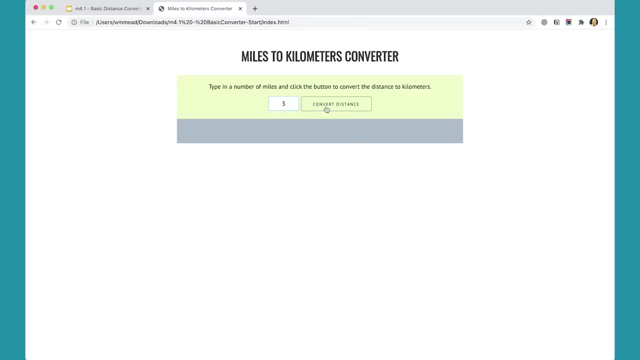 distance. we should get that data coming up here. so if I come back here and refresh this and then type in five and click convert distance, you can see that the alert pops up and it gives me a five. if I put 54, it'll come up and it'll give me a 54. 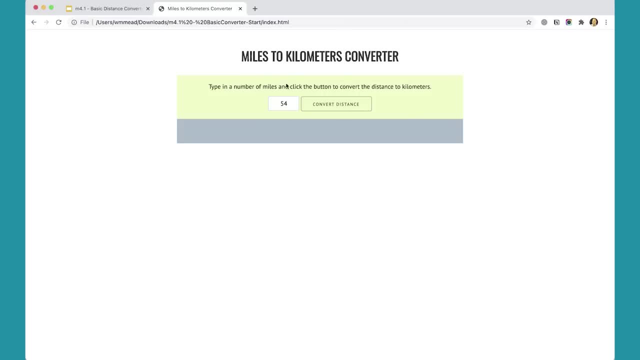 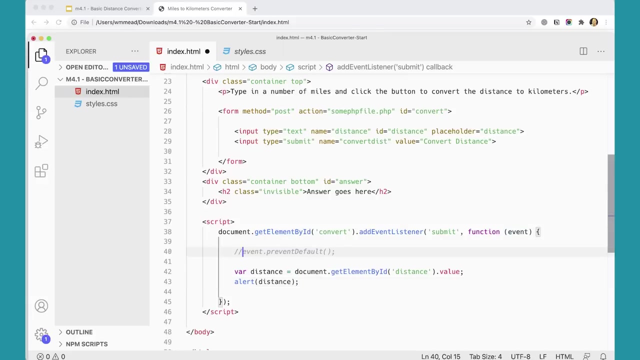 so that is capturing that value. it's preventing the default behavior of submitting this form and trying to go to the PHP file if you don't do event prevent default. let's just see what this happens for a second here, if I just comment this out and come back here and refresh this. 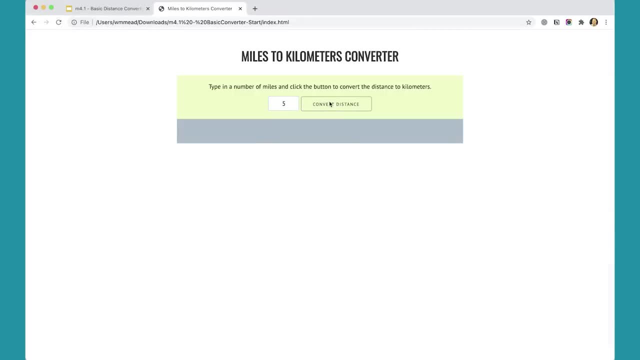 if I don't do prevent default convert distance, it gives me the five but then tries to go to some PHP file which we don't want. so it is getting that data, but then it's trying to go through to the form. so we don't want that, we want. 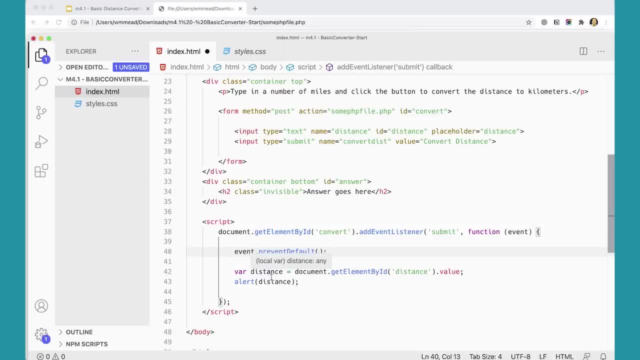 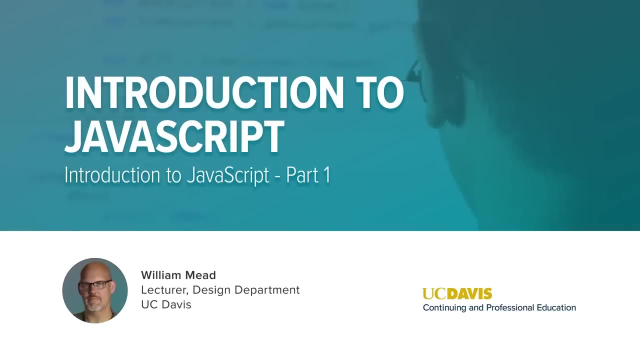 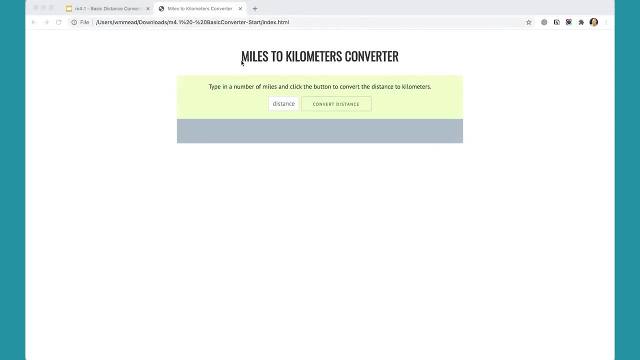 to prevent the default behavior, and that's what that does. okay, great. so we're getting that distance there and we're off and running here with our project. let's pick it up in the next video. the next thing that's important to understand is that when you type a number in here, 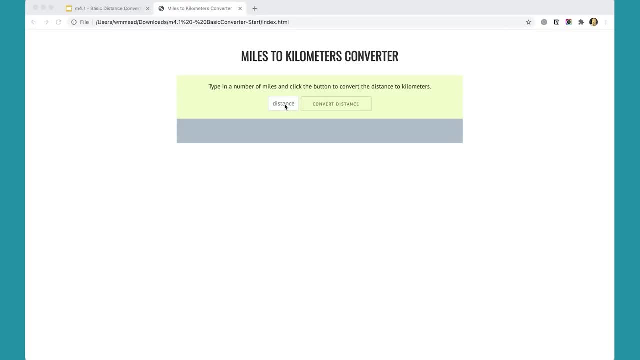 JavaScript sees that number as a string. so if I type a five in there, it'll be a string that holds the value five rather than the number five, and I need to actually take that number, that string, and convert it to a number. we could use a method. 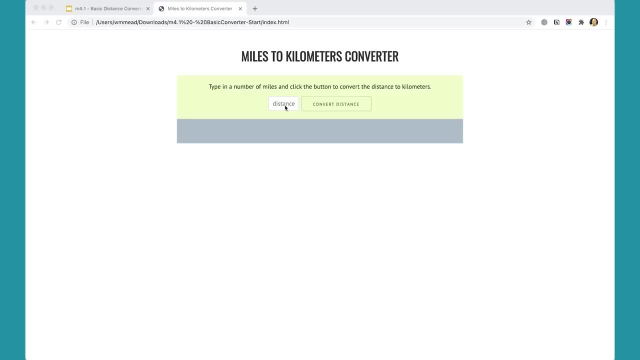 in JavaScript called parseInt. but what parseInt does is it'll only capture the integer of the number rather than a decimal number, and it's possible that I would want to capture the integer of the number and convert it to kilometers. so what we're going to use instead? 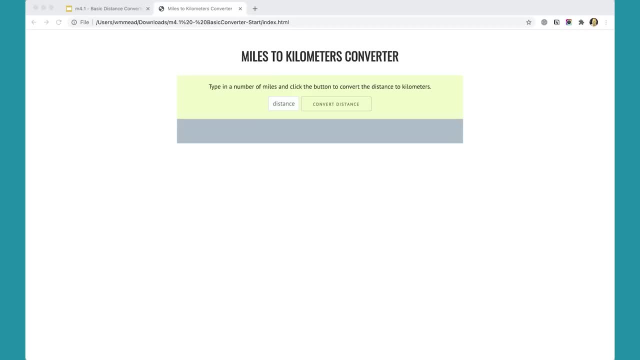 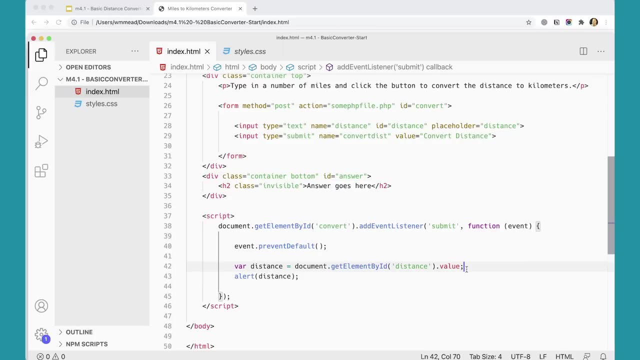 is parseFloat, and what parseFloat will do is it'll allow us to take that number and convert it to a floating decimal point. so down here I'm going to take, I'm going to leave the alert for a second here, but just before that I'm going to say: 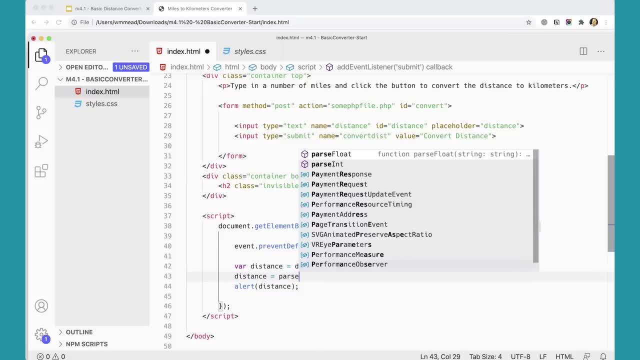 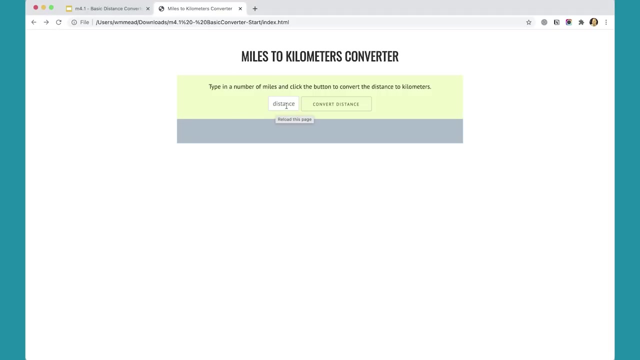 distance equals parseFloat. distance equals distance, so I'm taking distance and running it through parseFloat, then assigning it back to distance and I can alert that out. so let's just see what that gives us over here. if I come back and refresh this, if I put in a five, 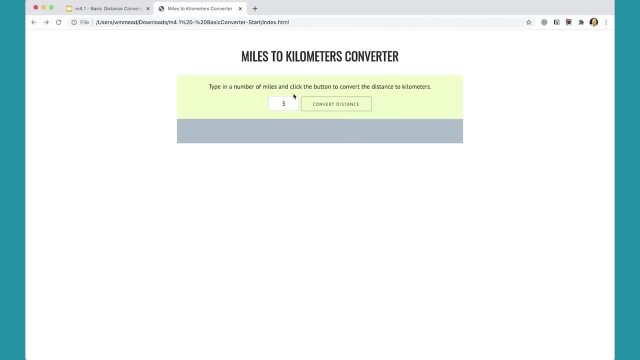 and convert distance, it'll give me a five, but if I put in chicken, it'll give me nan, not a number, which, as you know, resolves to false. so not a number is false, it's falsy, just like zero or a number of other things are falsy. 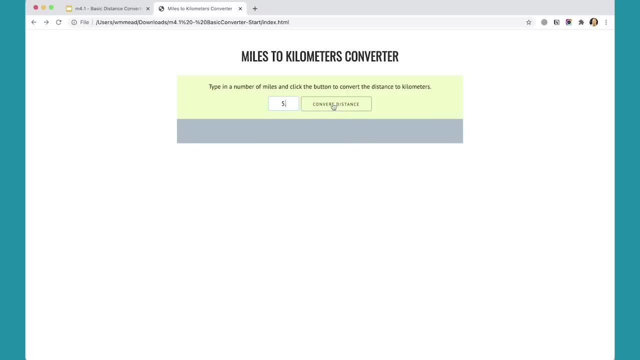 but a number is true. so five will work, 5.5 will work. interestingly, zero won't. zero is still false, but I don't know why you'd want to convert zero miles to zero kilometers, since they're both just zero. but that's what we need to do first. 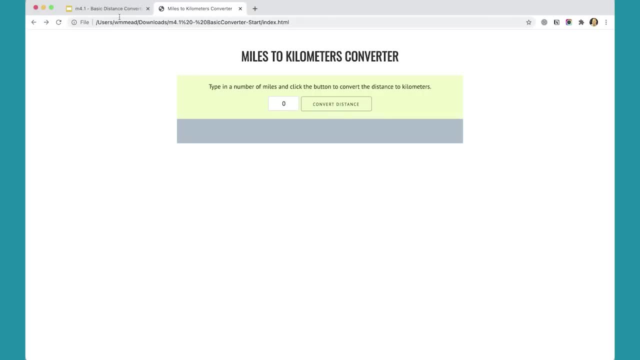 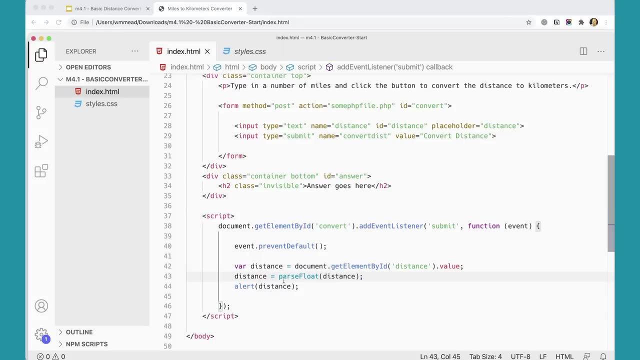 to get that to turn into a number now down here. we can actually combine these two lines into one line here, instead of having this distance and then assigning it back to itself. you could actually put parseFloat here with its opening parenthesis and we can close the parenthesis at the end after the value. 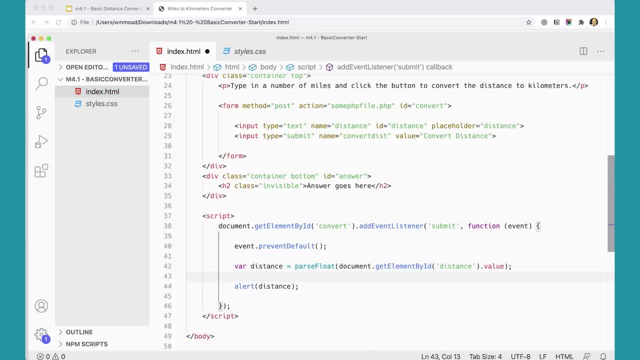 and we can get rid of this line. so that does the same thing all in one line. it takes the value distance from it, takes the value from the distance field and then runs it through parseFloat and assigns it to distance. remember, JavaScript works from the inside out. the next thing we need to do. 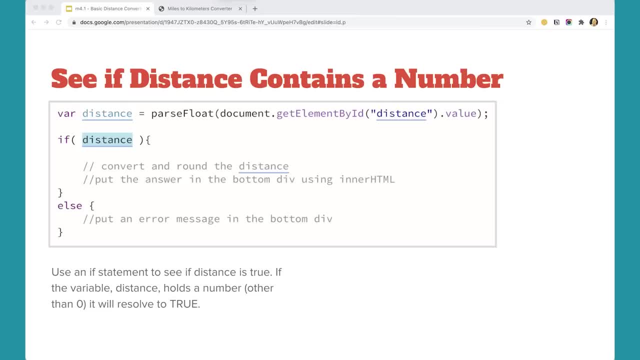 is check to see if distance is an actual number, instead of if somebody put in something that's not a number. we can't convert that to to kilometers, so we need to make sure distance is a number. so we can do that with an if statement and remember. 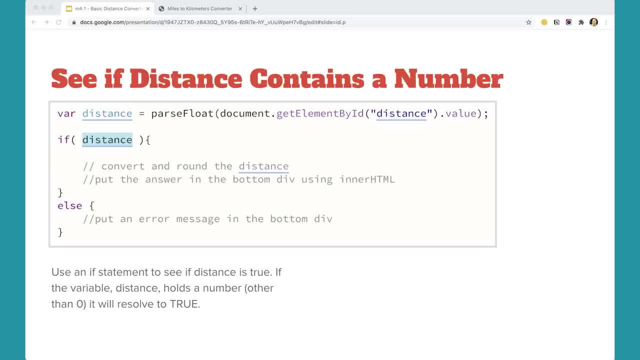 if we put in a number like 5 or 5.4 or 25 or whatever it is, that's going to come back true, that's true, that's truthy. whereas if you put something that's not a number that's going to parseFloat is going to convert it to nan, which is not a number. 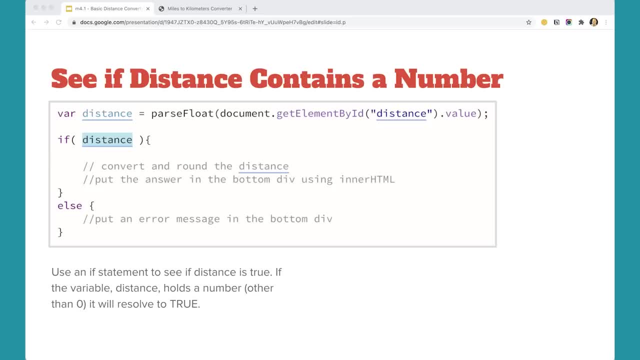 and that comes back false, or 0 will come back false, those kinds of things. so we can just say: if distance- so if distance is a number, because we're getting a number here- then we're going to convert and round the distance otherwise and then put the answer down at the bottom. 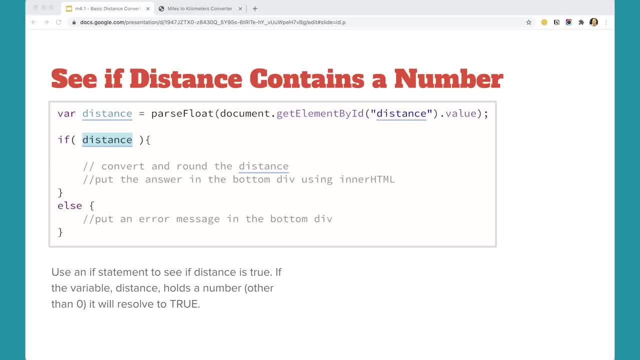 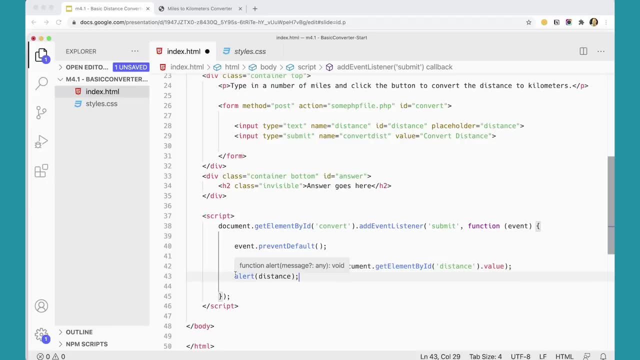 otherwise we'll display an error message down at the bottom. so let's go ahead and add this if statement down here- and we probably don't need this alert for right now, or I might end up moving it in a minute- if distance, we're going to do something. 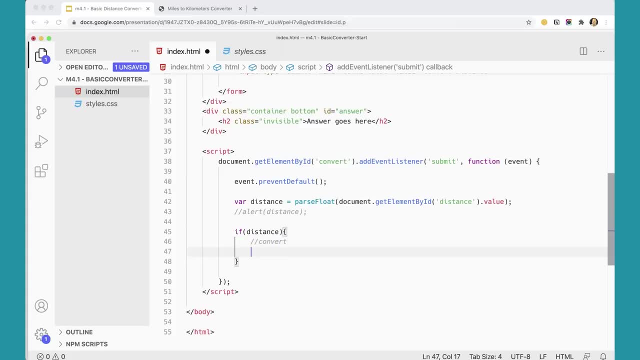 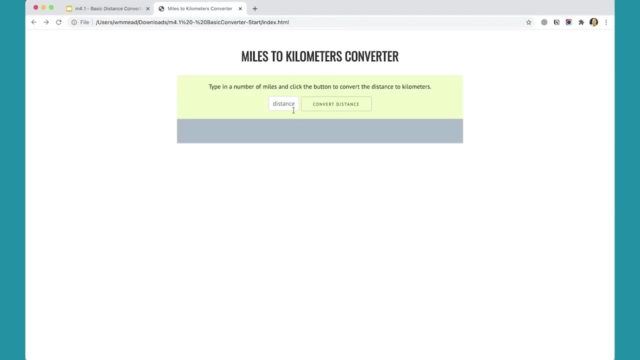 there. we're going to convert and then display the answer, else display error. okay, so let's actually take this alert distance here and stick it in here. we don't need it up here anymore. so you'll see now with that, if I test this, if I put a number in here. 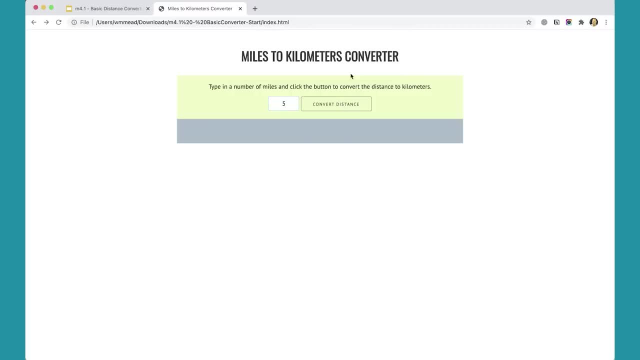 it'll alert out the number that I put in there. if I put something other than a number in there, it won't, because the else is running. we haven't actually done anything with the else, but it is running and it's not doing that alert. okay, great. 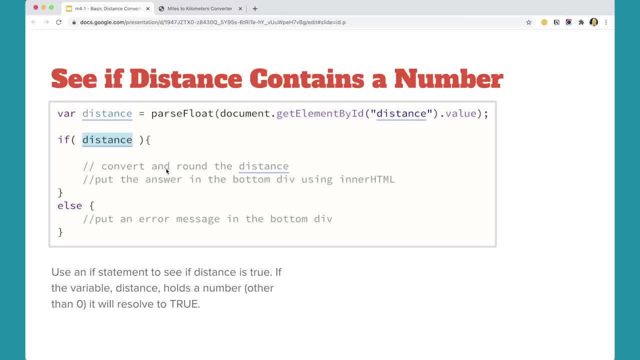 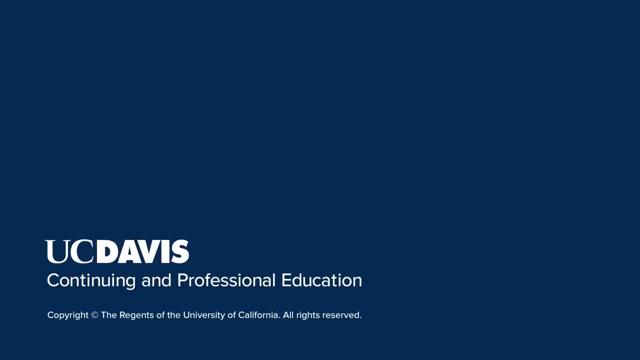 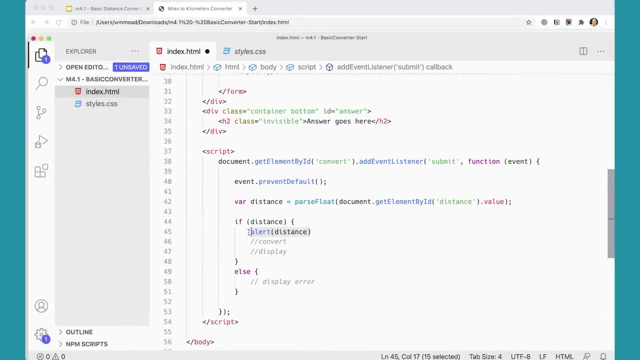 so we're all set up here and ready to write the rest of our script. let's go ahead and work on that next. so I'm going to make a variable here, get rid of this alert, make a variable rconversion, and I'm going to assign it. 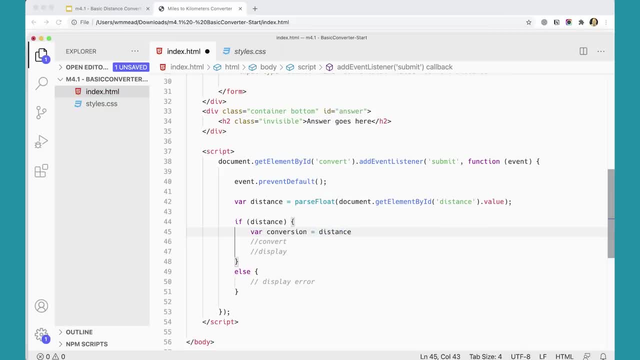 the conversion, which is distance times one point six, zero, nine, three, four, four, and what that will give us is the actual distance converted, but it's going to give us a very large number, or a number with a lot of numbers after the decimal point. potentially so, if I just 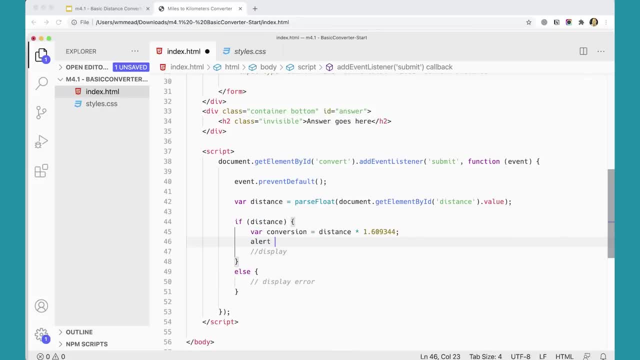 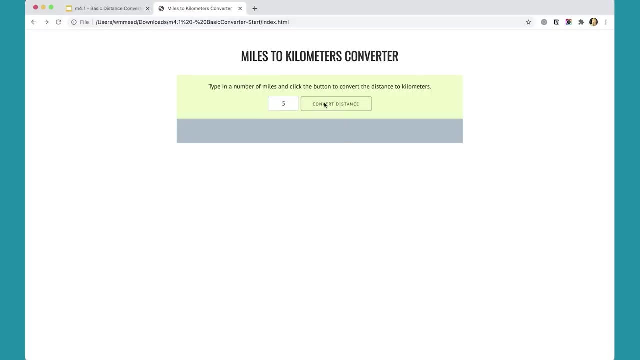 do here: alert conversion. make sure to spell that variable right and test that. you'll see what I mean if I come back here and refresh this. if I put in a five here I will get eight point. you know I don't want all these decimal numbers and I can get even longer than that. 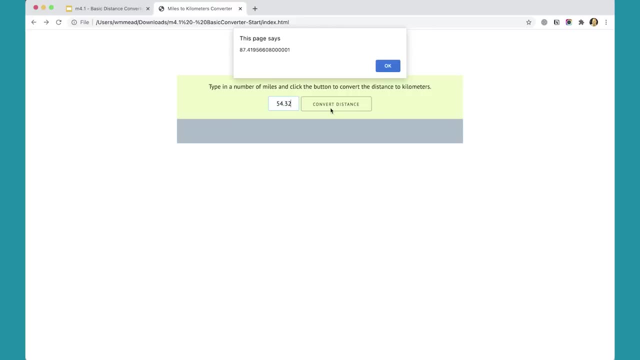 I did five point fifty, four point thirty two or something like that. you can see that's kind of long. I just want three here. I just want three. so there are a couple different ways of addressing this. in dealing with this, I'm going to show you kind of. 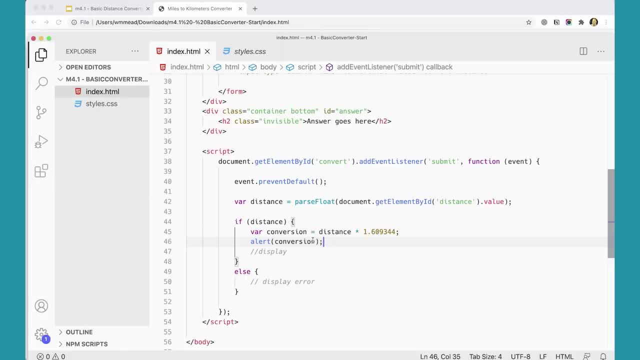 the manual way and then a way that's a little bit easier, because I think sometimes it's nice to see the manual way. so I'm going to make another variable: r two, two, two rounded conversion. rconversion equals math dot random, not random dot round math dot round. 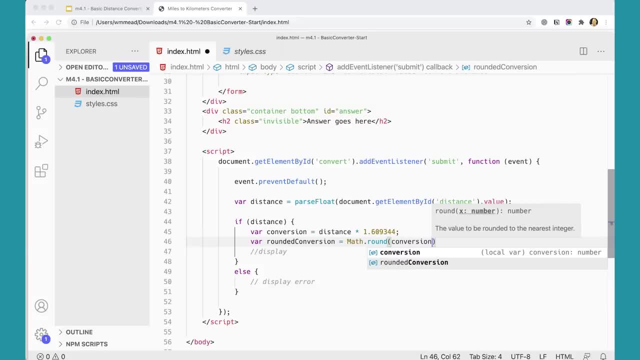 now, if I just put in math dot round conversion, what that's going to do is it's going to round it to the nearest whole number. I want some decimal points in there. so really what I want to do is I want to take that number and multiply it by a thousand. 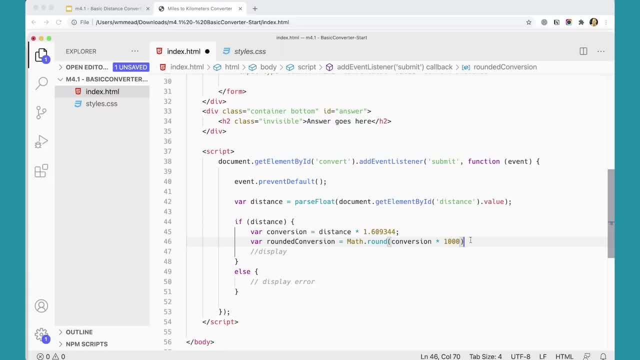 and then after the conversion, divide by a thousand. so that's going to take the number, round it and then divide it, and we might need an extra set of parentheses here just to make sure that it does the inner part first. so we round that, we take conversion multiplied. 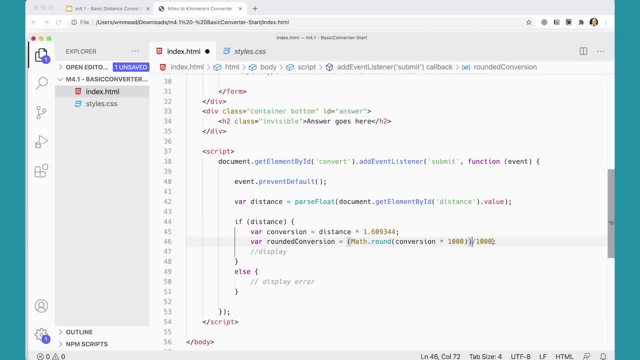 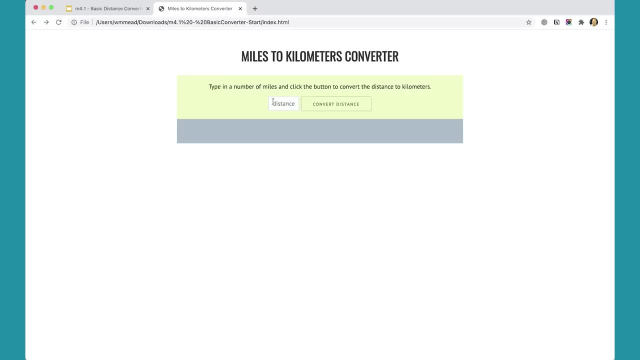 by a thousand, round it and then divide it by a thousand and let's see what that gives us. if we come back here now, if I try to convert this fifty four point three, two whoops, I have an error. let's see what I did wrong. there's always a good way to see. 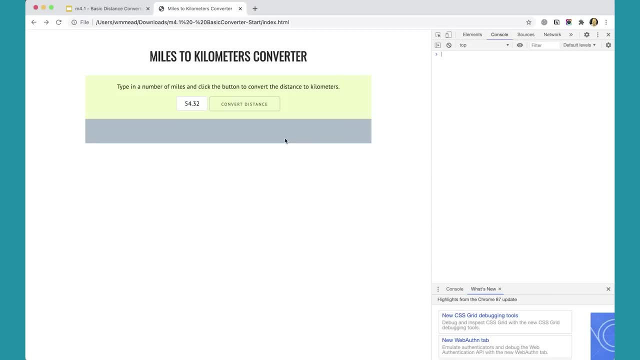 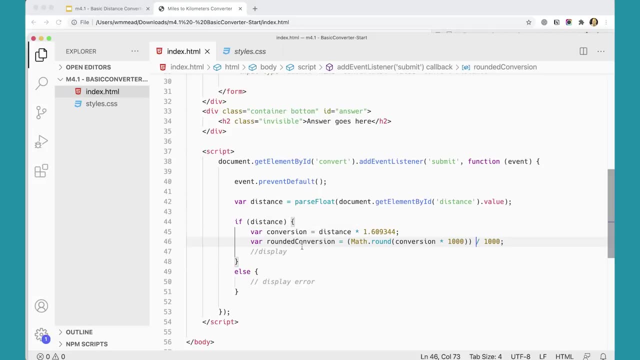 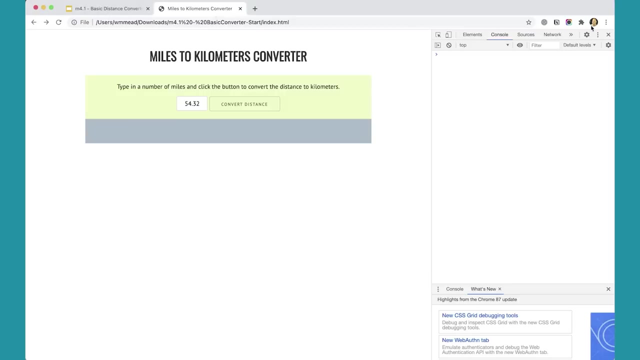 what's going on here? console or did I not actually do the? I forgot to do the alert. what's going on here? alert? rounded conversion. try that again. fifty four point three, two, convert distance and you can see that it's cropping it off here after two decimal places here. 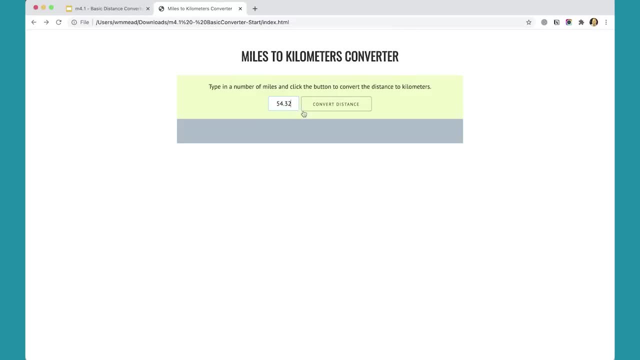 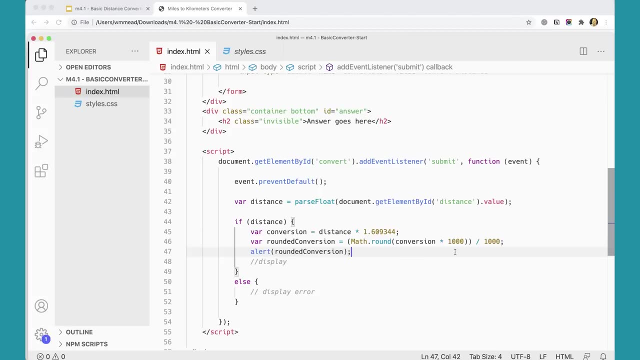 really more decimal places than that. the other thing you can do that's easier, a little bit easier than this, is to use um, something called two fixed. it's a method called two fixed, so I can take conversion and put two fixed and put three in there, and that will. 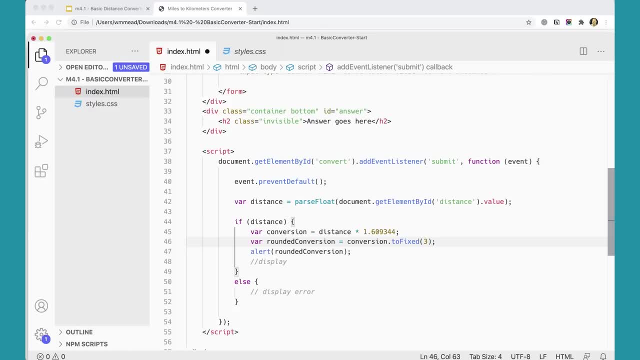 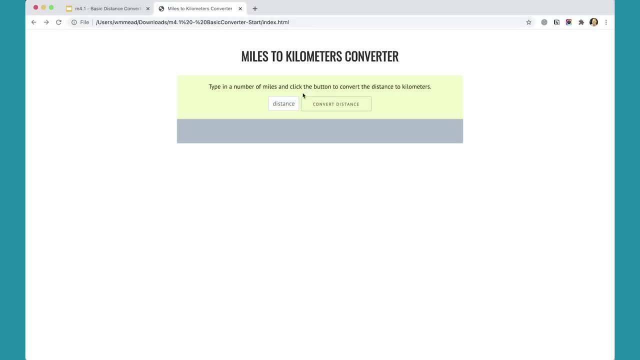 make sure it gets rounded to three decimal points. let's see what that does: fifty four point three, two, and now I'm getting eighty seven point four, two, zero, which is the right thing there. so that's actually rounding it and making it work exactly the way I want it to go. 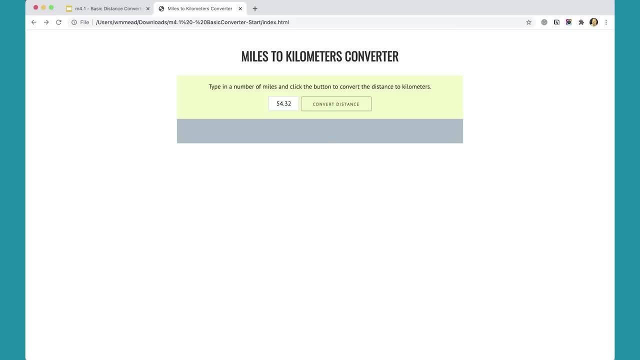 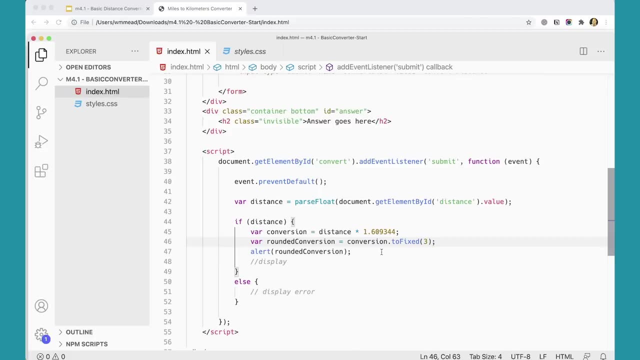 giving me three decimal points. so that's kind of the easiest method to work with. here is two fixed. now I can actually put this all together in one line also, so I could do a parenthesis here and a parenthesis there. so it does that first and then dot. 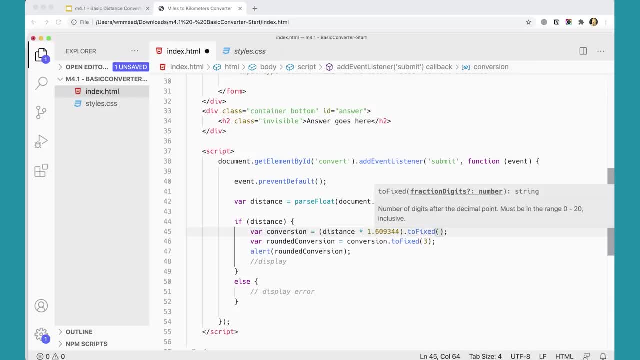 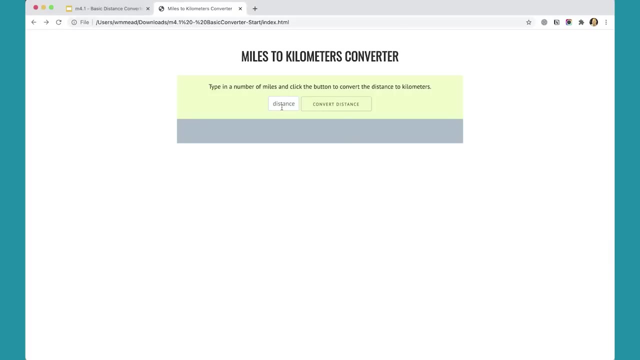 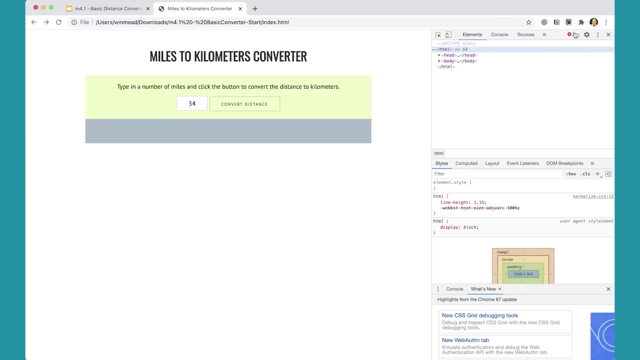 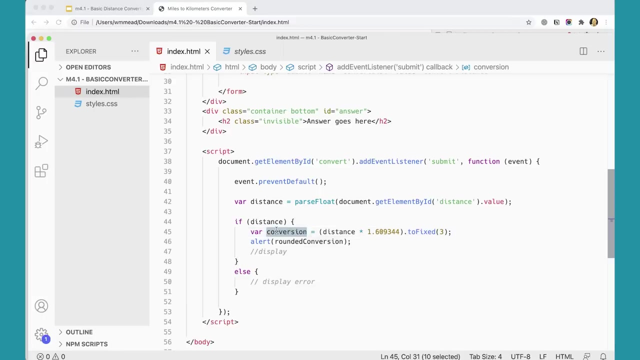 two fixed three and let's see. let's see if that works. fifty four convert distance. oops, I did something wrong there. now do I have any? and look, you can see I have any. console. rounded conversion is not defined over here. when I did this I needed to change. 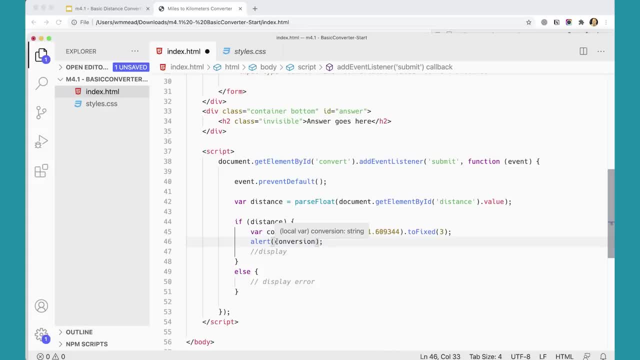 this variable here, so you can see how I figured that out. if it says rounded version, if it says a variable is not defined, you either spelled something wrong or you're using the wrong variable. let's fix that. that's a really good example of the kinds of things that 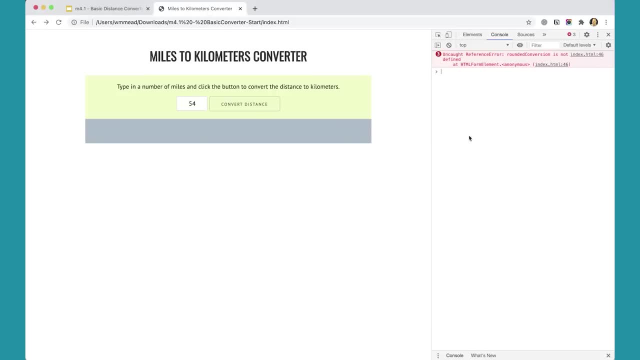 can go wrong. your inspectors, your friend, always go in here and see if you can figure out. sometimes the messages are a little obtuse, but usually with some experience you get to sort of see how that works. so there it is. that's working, just great. okay, cool, now we're ready to. 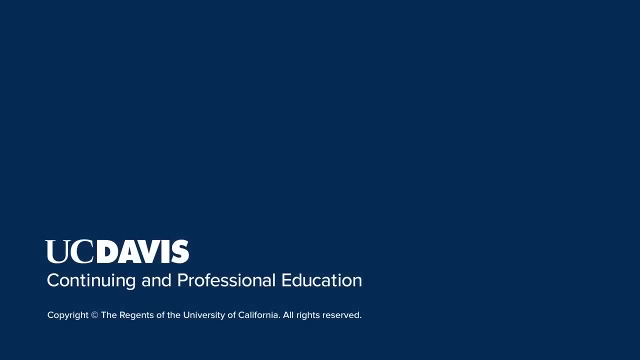 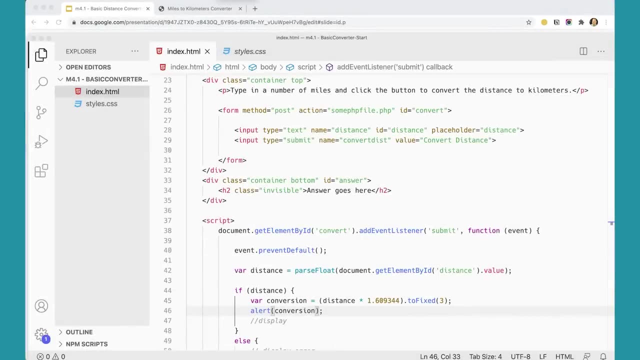 move on to the next part of the script. okay, one thing we want to look at really quickly here before we go on with the script is at this h2 down here. so right now I have an h2 in there with a class of invisible, and if you 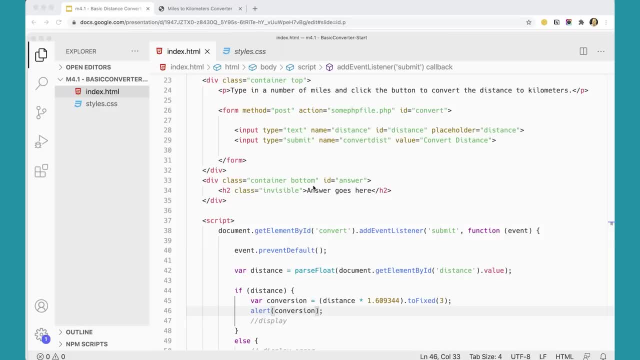 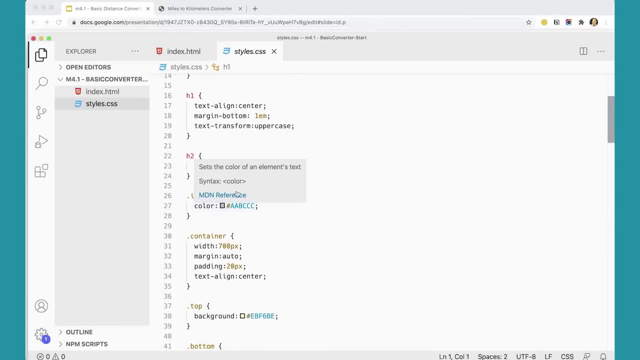 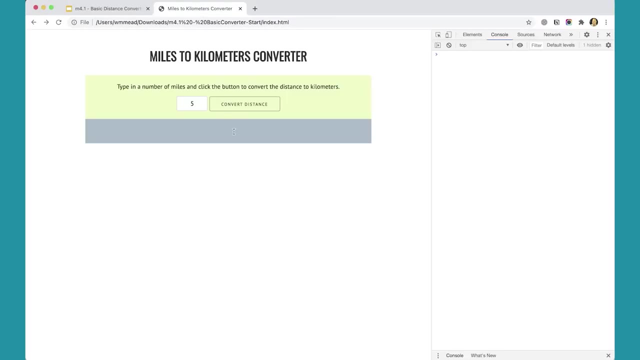 go look at the styles, you'll notice that this class, invisible over here in the styles, is doing something to make that. it's basically setting the color of that text to the same color as the background of this div and over here, if you go and actually look at this thing, you'll notice. 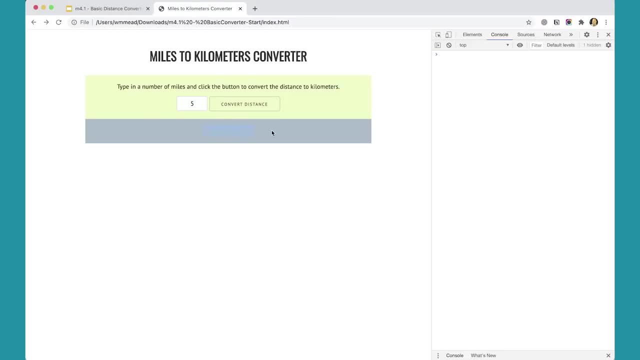 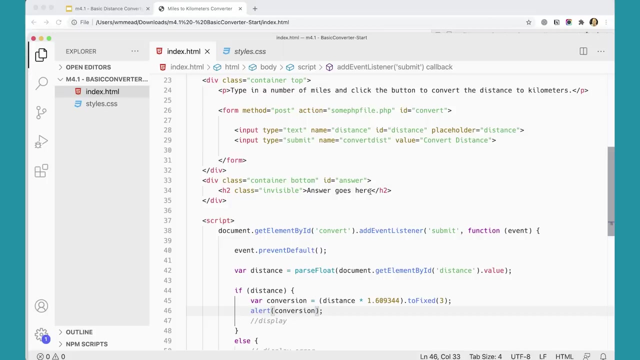 down here that that answer is in there. it's in there. you can't really see it because it's the same color, but it's actually there and it just says currently. what it says is: answer goes here. but what we can do is we can use inner html to: 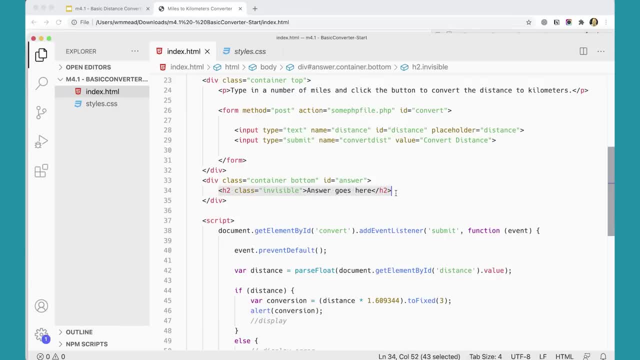 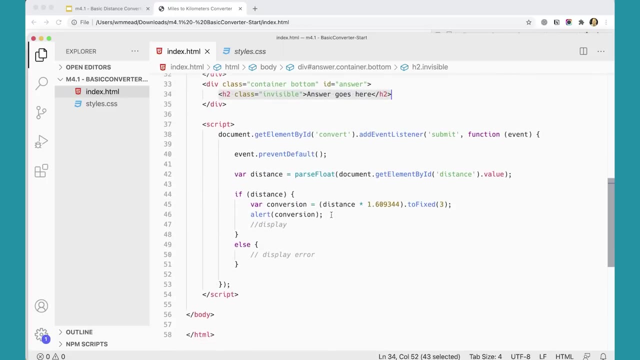 replace this entire h2 in here with a new h2, and that h2 that we put in there won't have the class invisible, so it will be visible. so we want to get this div id answer here first, so up here let's get rid of this. 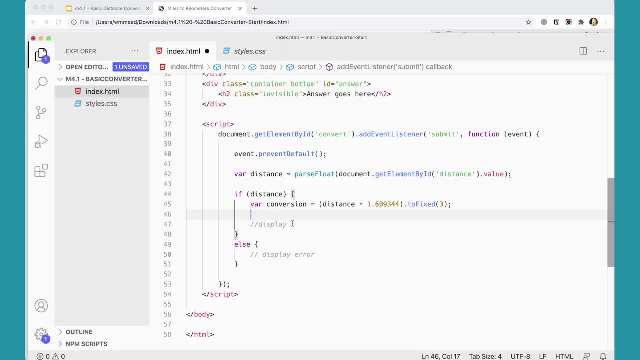 alert. we're going to work on this display piece here, so let me get rid of that. so first thing I'm going to do is I'm going to have a variable var answer and set that to equal to document dot. get element by id answer answer. that's our. 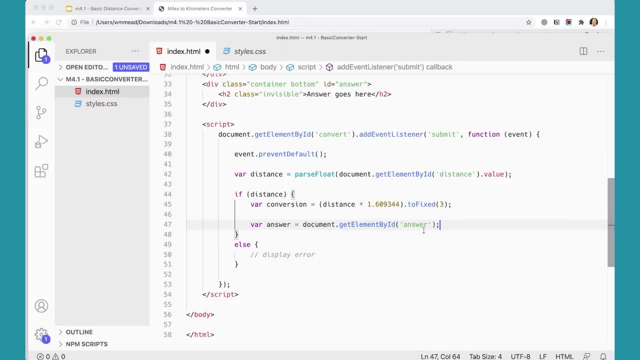 element there that we're getting, and then we want to get that element and and we want to use inner html. so I'm going to say: answer dot. inner html equals quote, quote, and in here I'm going to add an h2, h2 which opens and closes. 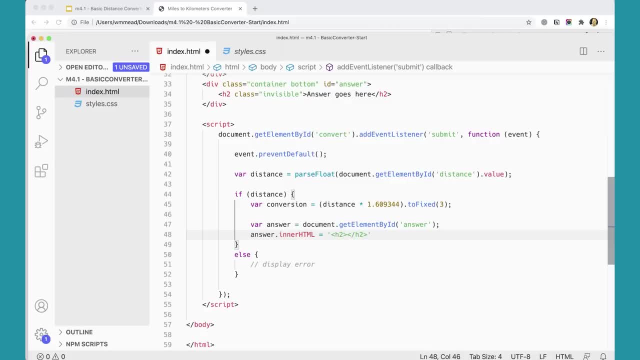 h2. it's always best to open and close things right away. and then in here I'm going to say, actually, rather than use the quotes, here I'm going to use the tick marks. so, like that semicolon, let's do that again. h2- close the h2. 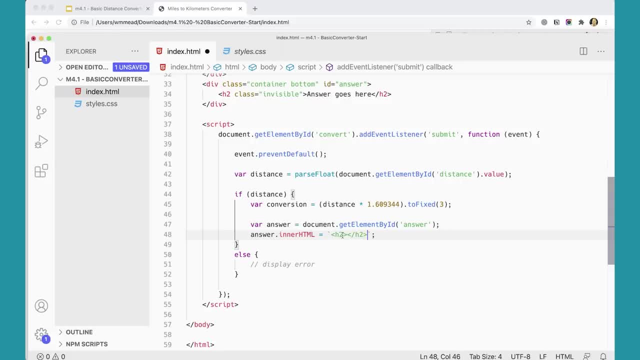 there we go, because this is going to be a string, literal when we're done here. okay, so in here I'm going to add, um, the uh distance. let's see what do I want to put in here? I want to put distance in here. distance miles converts to: 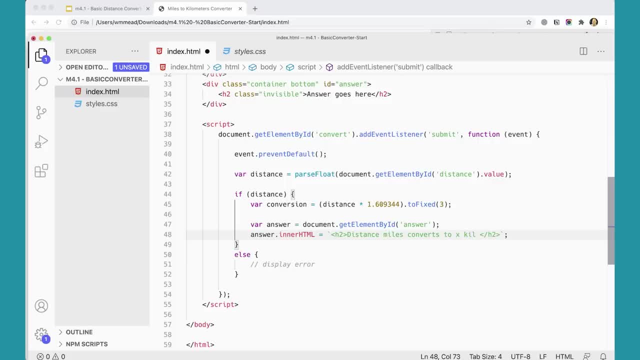 x kilometers, right, where distance is really this variable distance here? so that's going to be a variable. so in there I'm going to put curly braces dollar sign, curly braces distance, because that's a variable. miles converts to, and x is going to be dollar sign: curly braces. 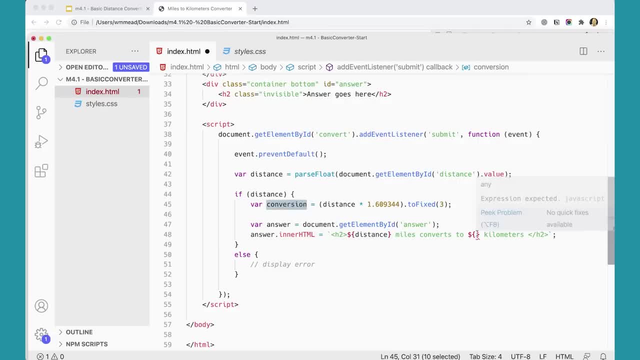 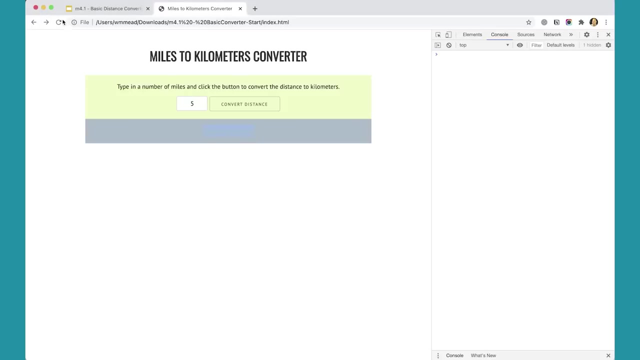 conversion and stick conversion in there and and that should actually work. so let's see if that actually works. come back over here. if I refresh this page and put a number in here and click convert, you can see five miles converts to 8.47 .047 kilometers. 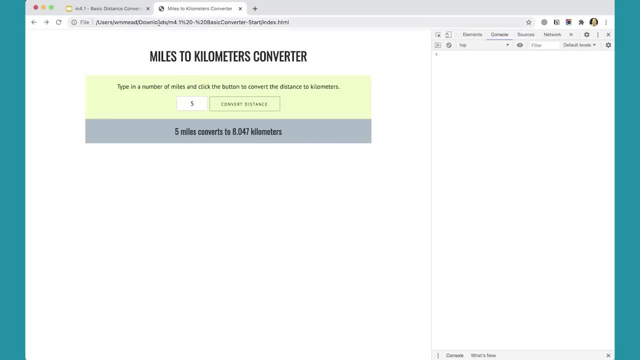 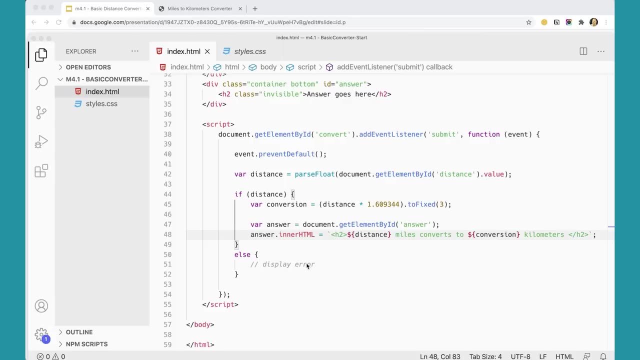 and so that works perfectly fine. that's great. the next thing we need to do is handle the error down here and we're going to put it into the same element here, this answer element here, so I could use document, document, dot, get element by id and go. 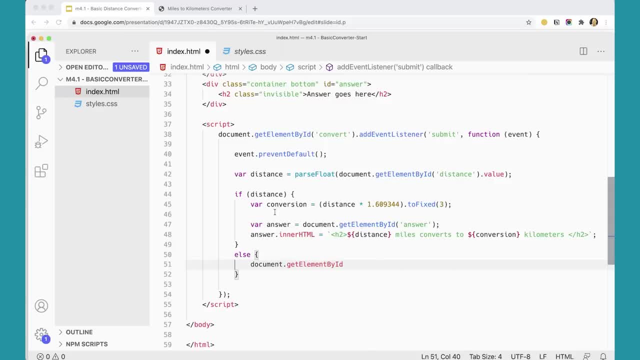 get this answer div again and use inner html again. but since we've already gotten this and put it into this variable here, it makes more sense to move this variable out of the if statement and stick it up here somewhere. go anywhere, really, I'll stick it here. 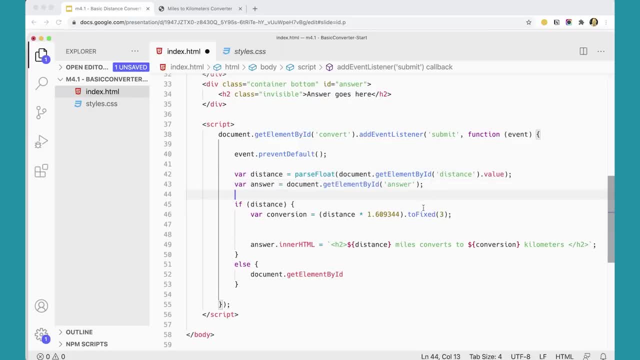 so that's going to get defined to begin with. it could even go after the prevent default. it could go anywhere really, but I'm going to just put it there and then I can use the exact same variable down here. answer dot. inner html equals. and now I don't have to use the tick marks. 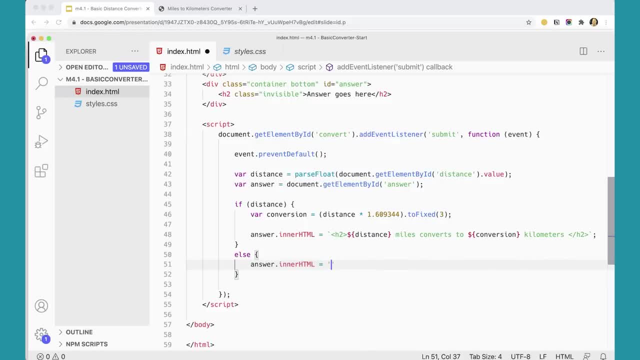 because I'm not going to pass any variables in here, so I can just use regular quotes- h2, close the h2, and always open and close before and then work on the inside from that way, please provide a number so that will handle the error. so let's. 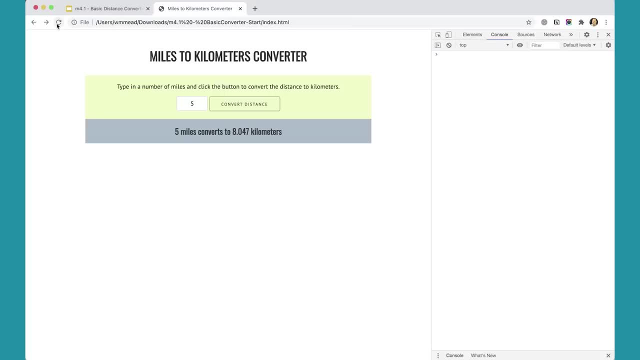 make sure that works. we come back over here and refresh this. if I put a chicken in here, a chicken cannot get converted to kilometers. so it says: please provide a number. but if I put a number in here, that will convert, just fine. so our our little converter. 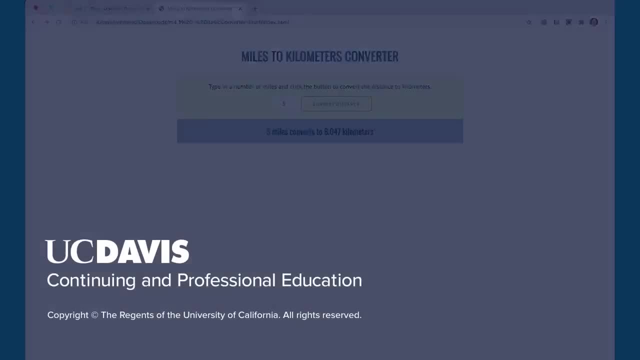 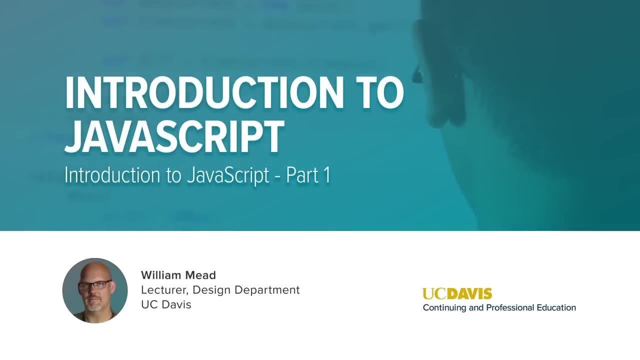 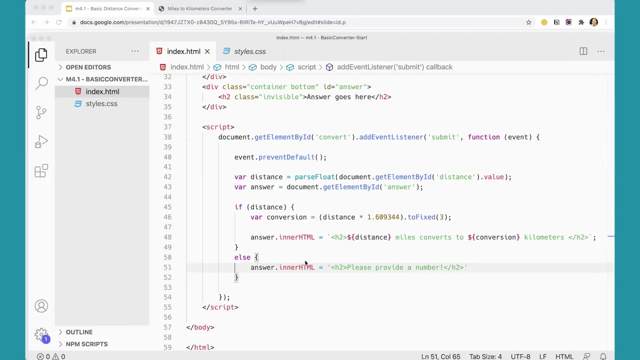 is working great and that's awesome. this is our entire script and it's working pretty well. at this point it seems to be working fine and we've done a little bit of refactoring to kind of get it to a little bit more compact and a little bit more readable. 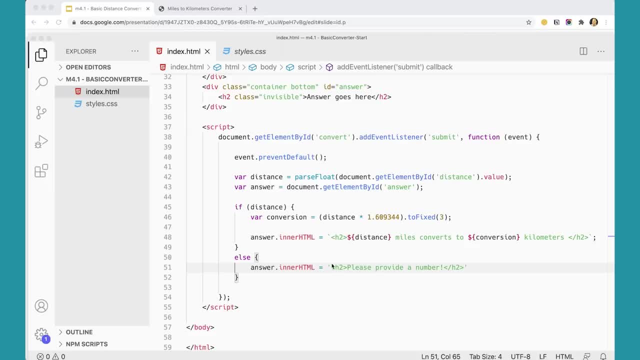 we've tried a few different methods to make that all work, and it's all working great, and we could leave this script at the bottom of the page. there's not that much to it and it's fine, but just for the sake of practice, let's move. 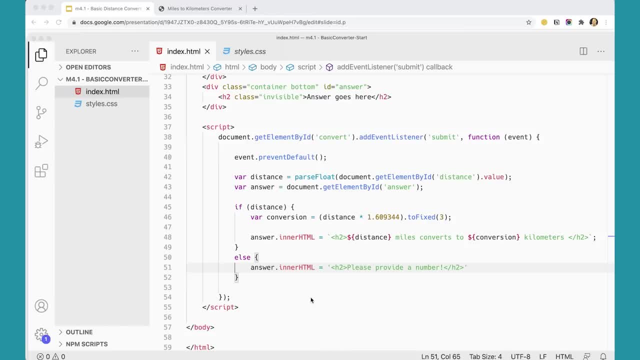 it to an external file and link it up and then use our scope and best practices for converting everything. so over here I'm going to, I'm going to come over here I'm going to make. oops, I didn't mean to make a folder, I'm going to make a. 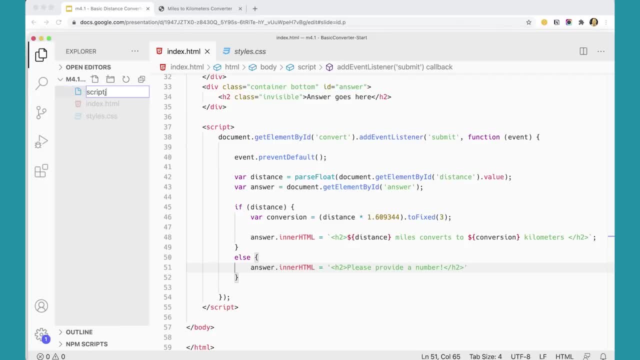 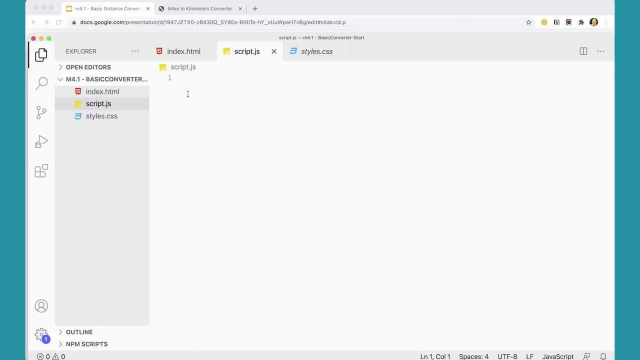 file and call it script dot js, and on that file I'm going to add my iife, my immediately invoked function expression, so that starts with parentheses. and then in there I add a function with its parentheses and its curly braces, and then another set of parentheses and a semicolon. 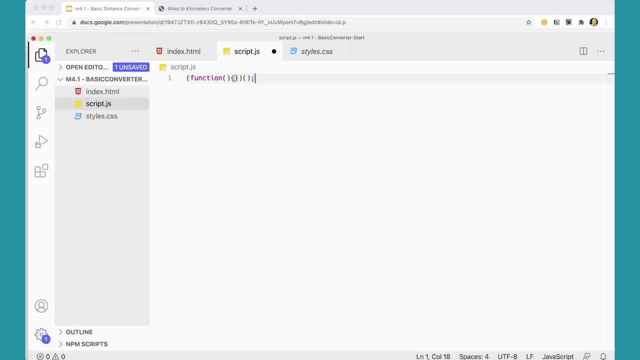 so this thing will run: when the page, when the script, when the script file loads, it'll run. and my script is going to go inside the curly braces. so I'm going to move those down and also I'm going to add in here: use strict, my use strict directive. 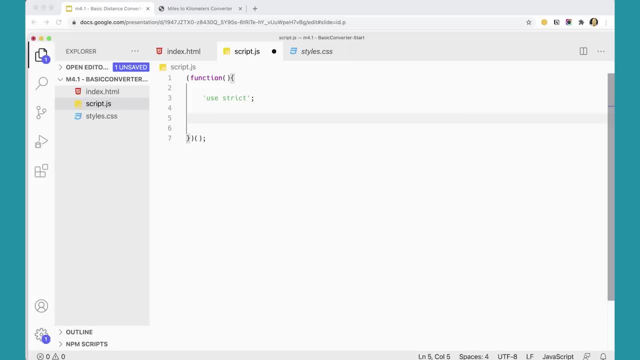 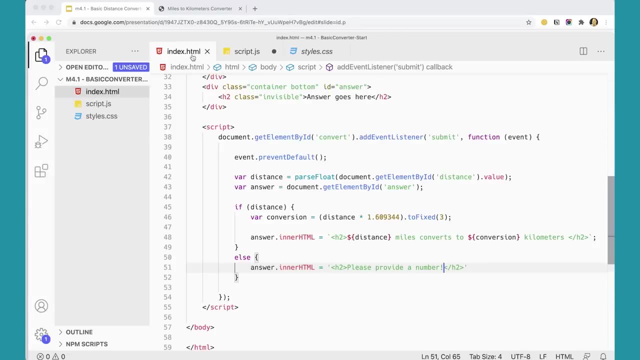 which is going to make sure that I'm not defining any variables without the var keyword. they don't get put into the wrong scope. I don't really have to worry that much about scope here, since it's all pretty much within this one event handler, but still it's a good idea to put it in. 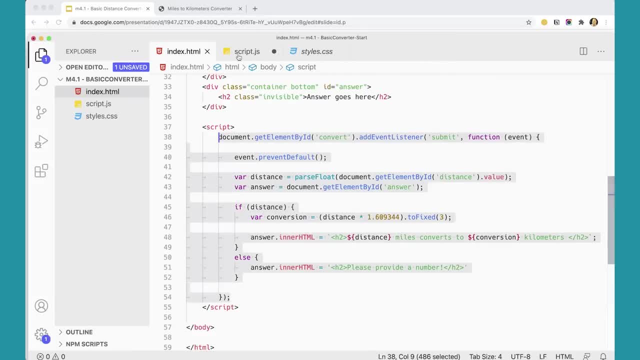 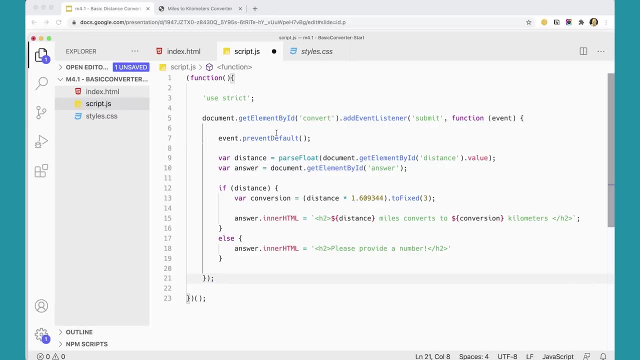 so then I'm just going to copy all of this stuff, or you could cut it and paste it over here. there we go, there's our script, and in here I'm going to come in and change my vars to either const or let. I think they will all work. 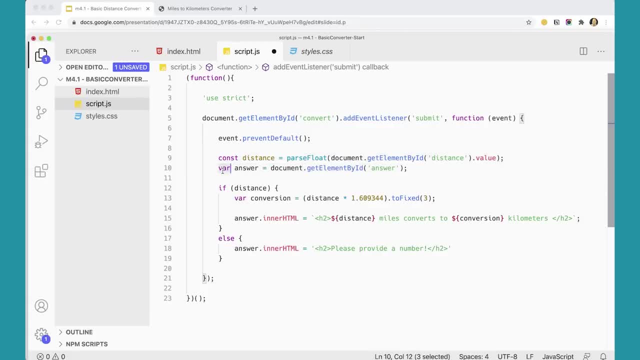 with const. distance is going to get that once and distance is not going to change. const is going to come down here, answer is always going to be answer, and then this one here, const as well, conversion. so we've got all of that set. alright, great over here. on my HTML file. 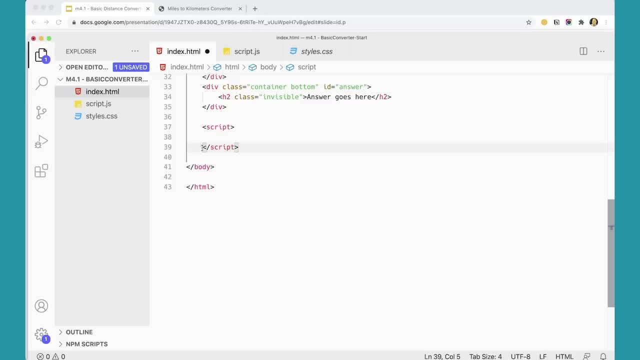 instead of having this script here, I can leave it at the bottom of the screen if I want, that's fine, and just link to it here. src equals quote script dot js, and that should work just fine. so if I go ahead and test that, it should work exactly the same. 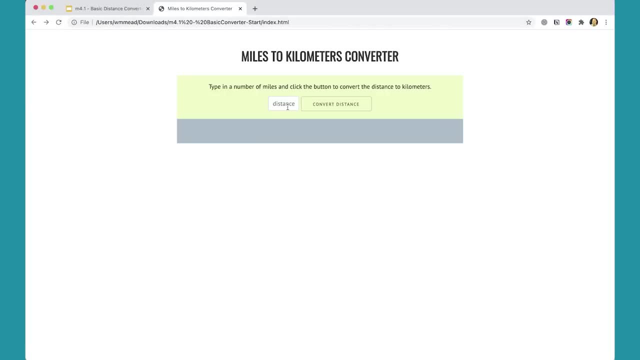 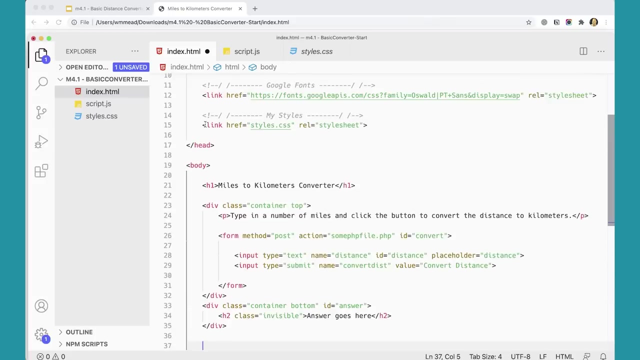 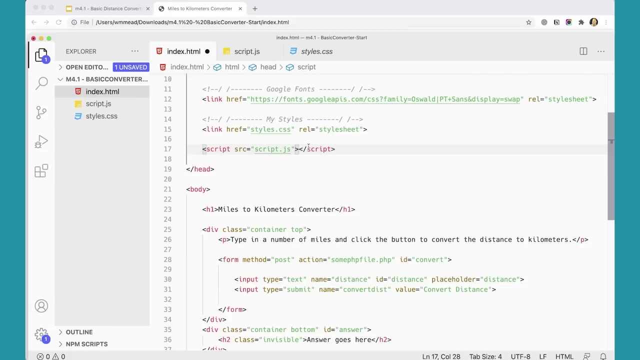 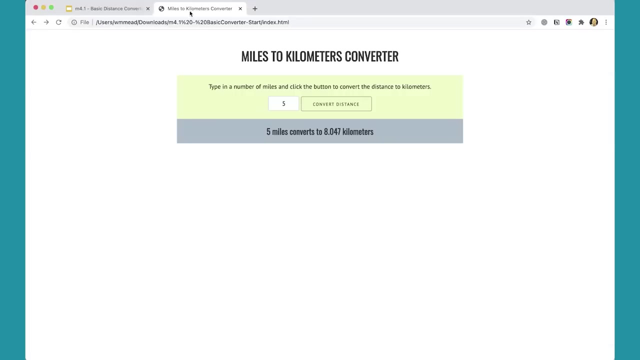 as it worked before and it works fine. that's great. now I could also move the script up into the head of the page, up here into the head, but I have to add the defer attribute here: defer- ok, and if I come back and test it, you'll see that still works. 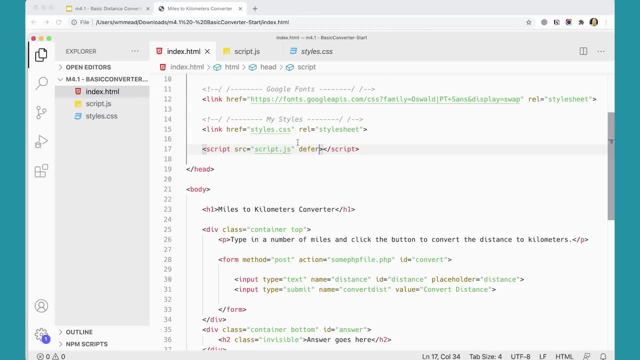 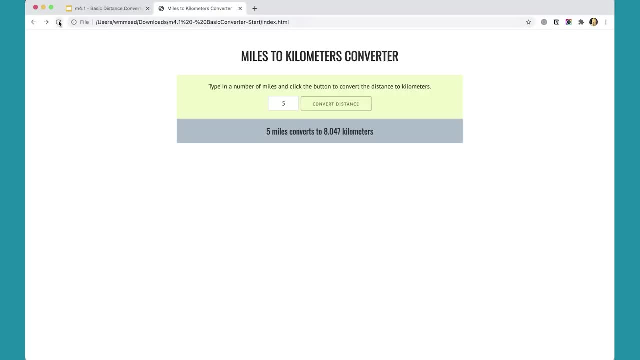 if you forget the defer attribute up here, then it's going to try to run that script before the page loads and it won't work properly. your file is trying to go to the sumphp file because that script never loaded and it never prevented the default behavior. 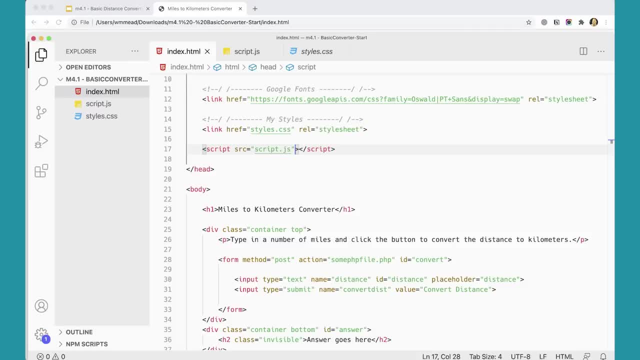 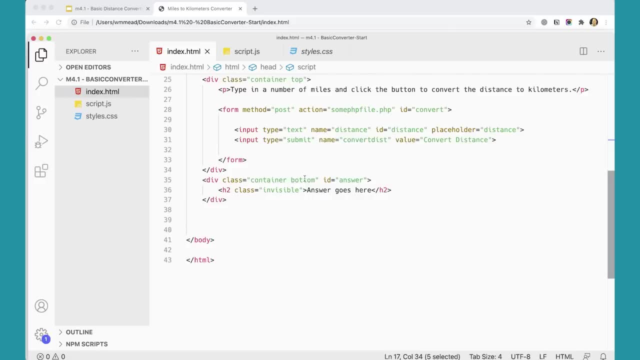 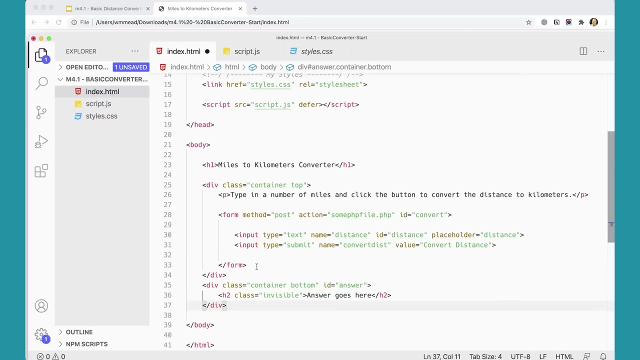 so that didn't work. so you need to have that defer keyword in there to make sure that this script is deferred until the rest of the file loads. but there we have it. it's a great little tool and it's allowed us to practice many of the things. 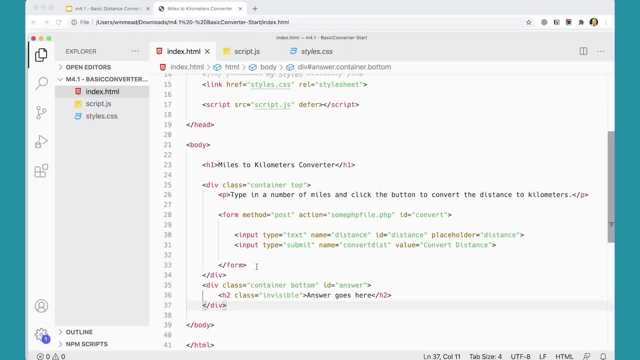 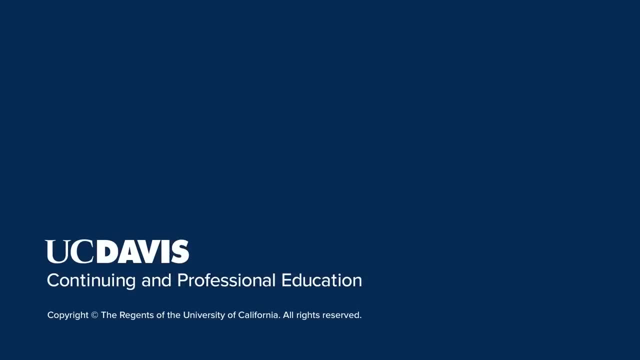 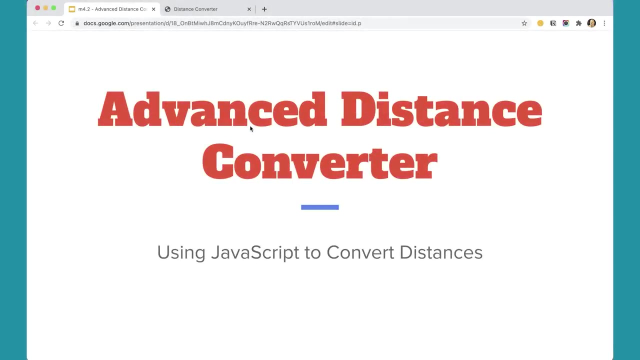 that we've been talking about during this course and we'll look at a slightly more advanced version of the project. next, advanced distance converter: using javascript to convert distances. in this project we're going to use an extension to what we did in the earlier project for the distance converter. 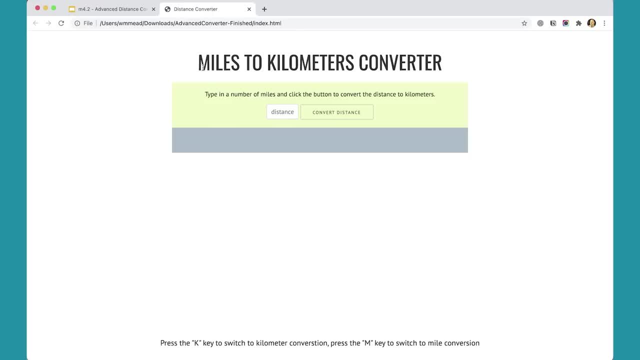 we're just going to add an additional feature, and what that additional feature is? it'll convert miles to kilometers. but we can press the k key to convert kilometers to miles or we can press the m key to go back, so we can go back and forth between doing different types of conversions. 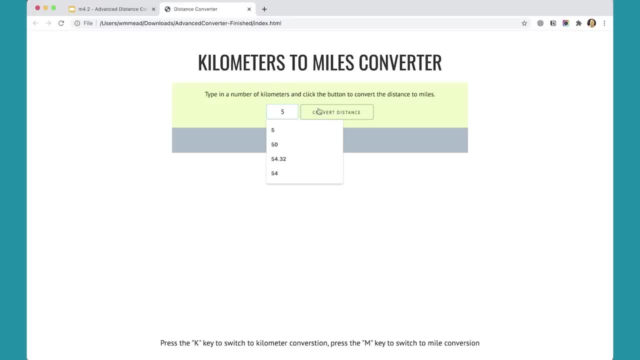 so that's kind of neat. so if I put a 5 in here and click convert distance, it'll tell me 5 kilometers converts to 3.107 miles. or if I press the m key, I can convert 5 miles to 8.047 kilometers. 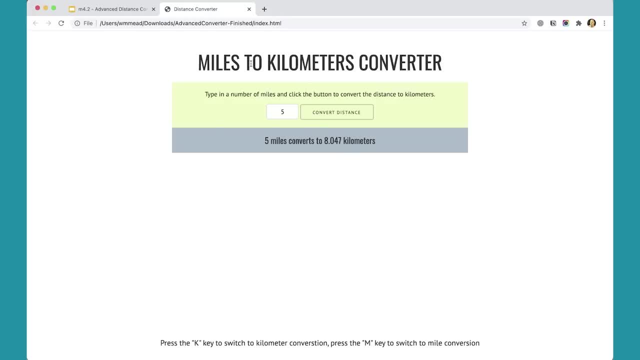 so that's pretty neat. notice that a few things are changing when I do this. the header changes here, this little piece of instruction changes slightly here and a few other things have to be managed down here. I've got a set of instructions down here on the bottom of the page. 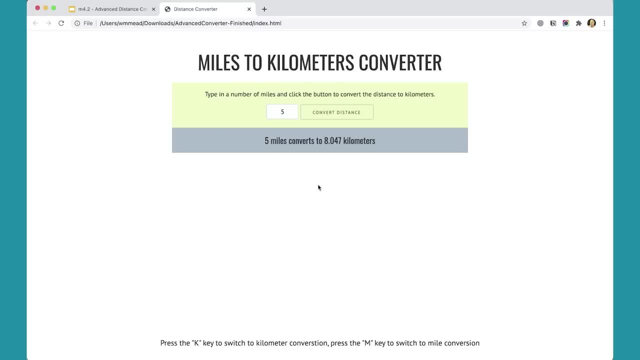 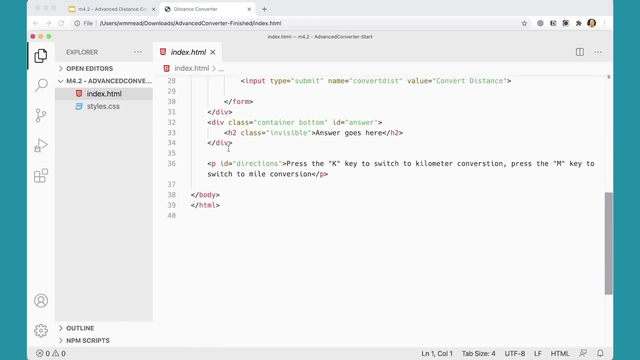 that tell you which keys to press and that kind of stuff. so that gets us set up to start coding this project and getting the script working. and you'll notice that if you look at the start file here, it looks very similar to what we had before. we just need to. 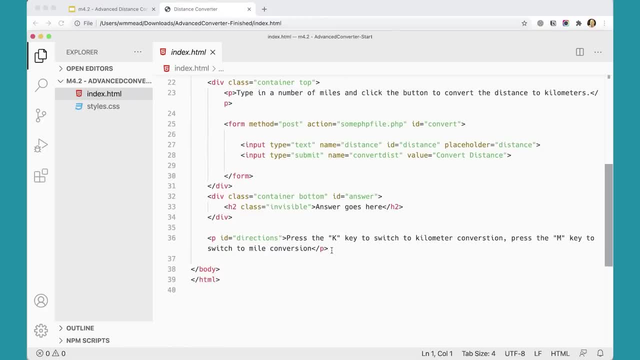 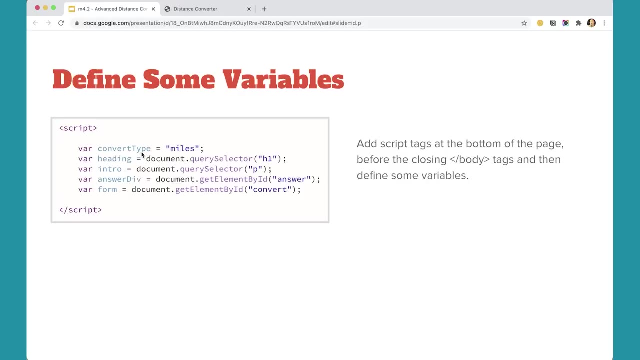 get started with a script tag down here, and then the very first thing we're going to put in there is just some variables that we need in order to make this work. we're going to need a variable called convert type that's going to be set initially to miles. 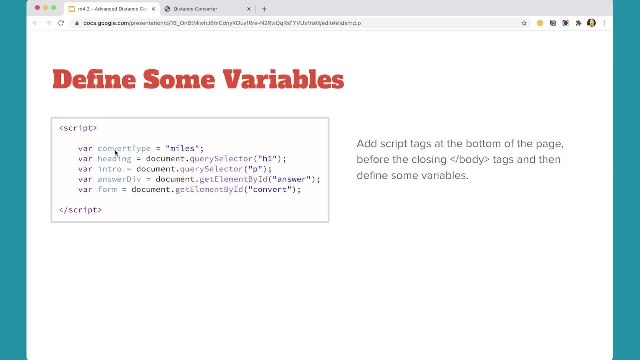 and then when you press the k key or the m key, it's going to update that value to kilometers or miles, depending on which key you press. so we'll be capturing key presses and doing that kind of thing. so let's do that. and then we also need to get the h1. 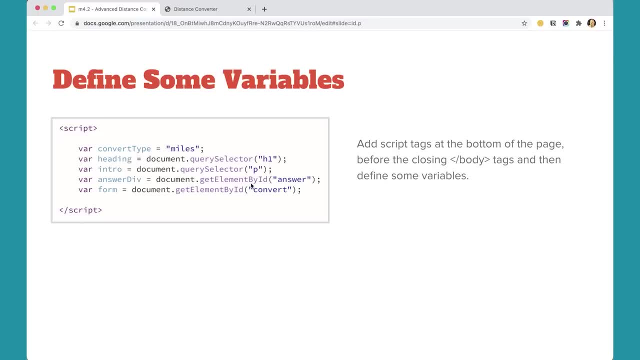 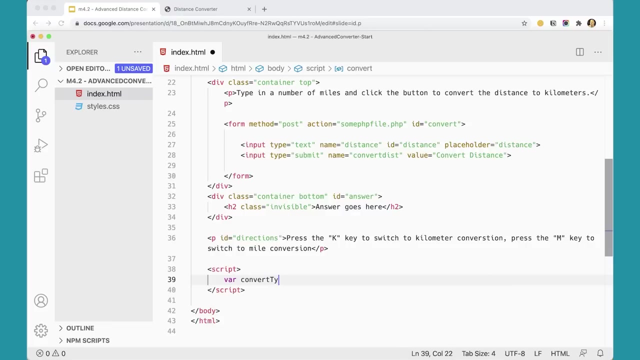 because we're going to change that in the intro text. we might as well gather that answer element down there as well. that we have in there. so let's go ahead and add these variables really quickly. var. convert type. I'm going to set it to miles initially. 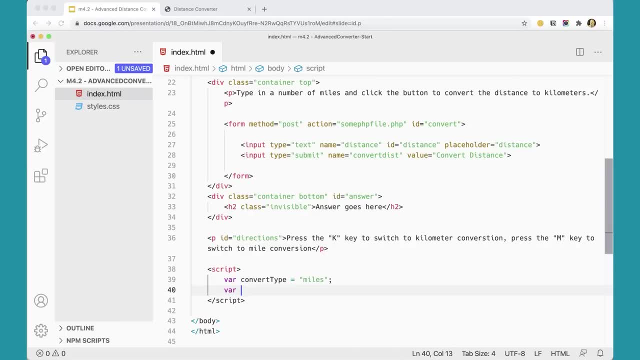 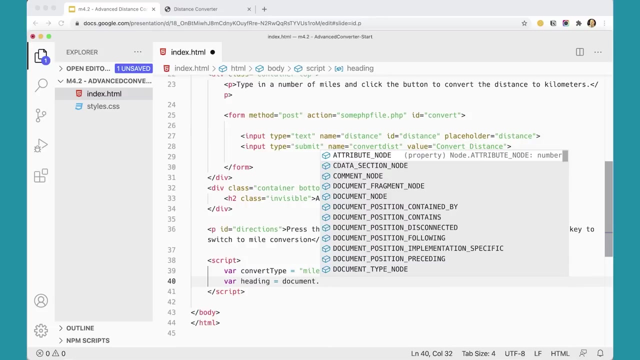 and then I've got var and I've got what did I call it? heading? heading yup or heading equals document dot get element. we don't have an id up there, do we no? so I guess we should use query selector. query selector h1. 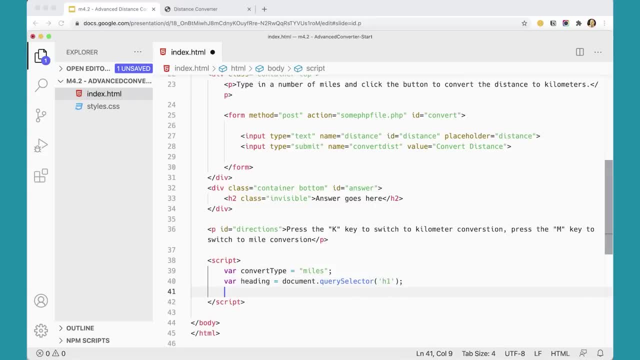 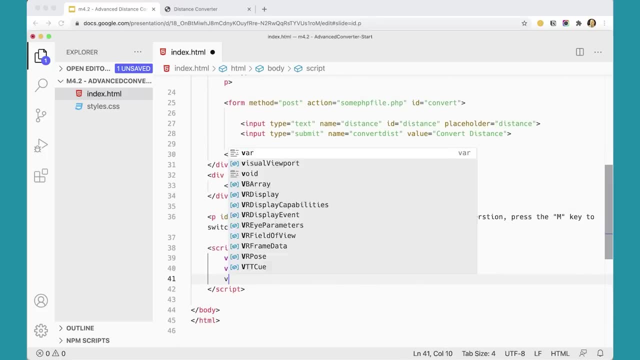 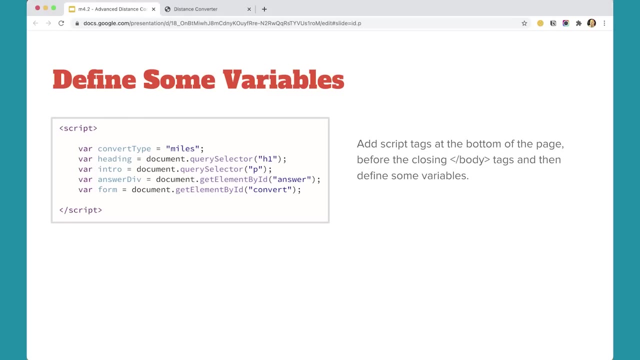 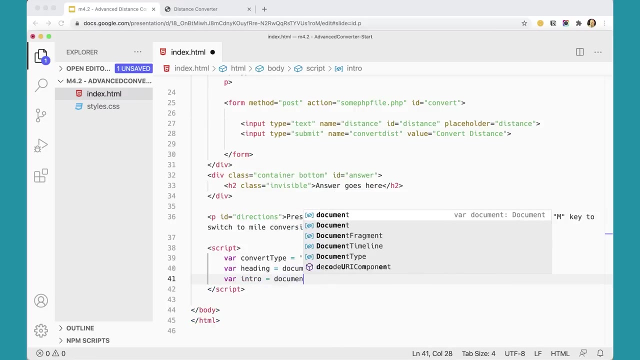 that will get the heading, and then we need this sort of intro paragraph here. so var and just to make it match what I have over here, it doesn't really matter, I'm just going to call it. intro. equals document dot. query selector p. this is the first paragraph on the page. 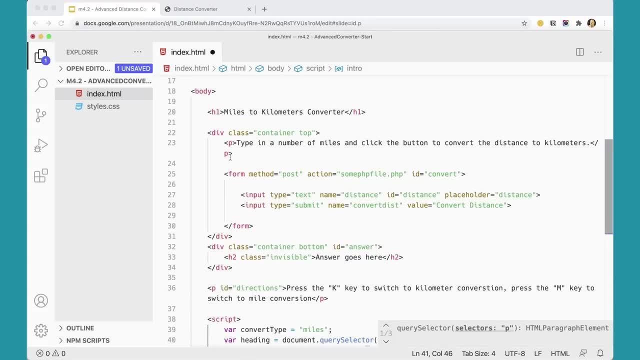 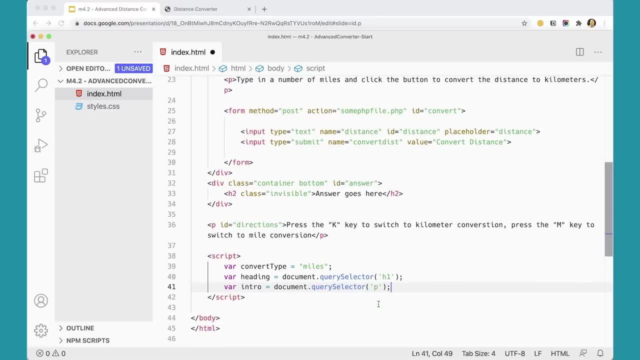 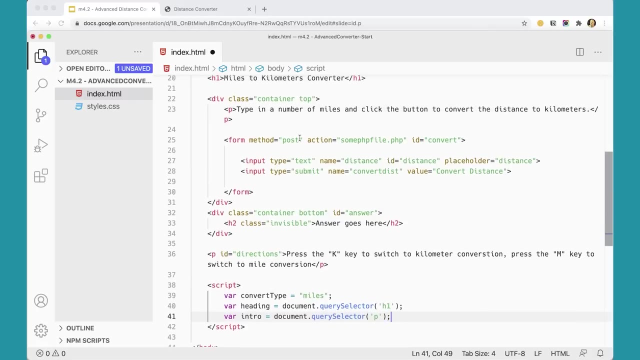 actually it's the only paragraph on the page, but remember query selector will grab the first one that it finds, so that's kind of handy. so I can just do query selector p. I don't have to do anything complicated to get to that paragraph. so we can get to that. 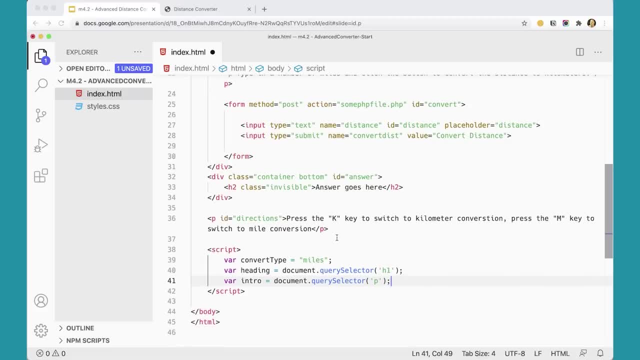 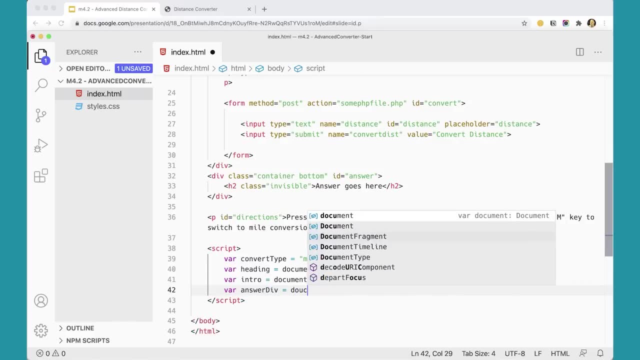 we might as well grab this answer div down here. var answer: div equals document dot. get element. this one I'm going to use get element by id and then I'm going to and the id I need for that is answer right, yeah answer. and then we might as well. 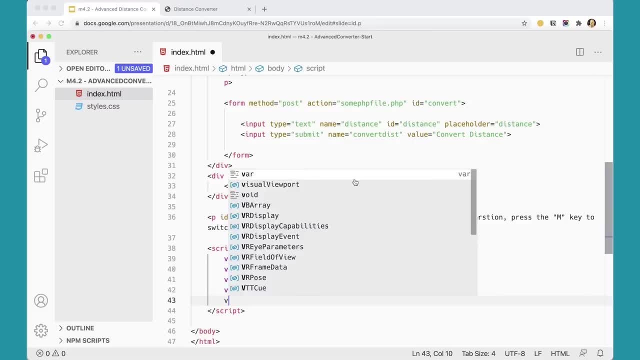 also get the actual form: var, form equals document, dot. get element by id and the form is as the id set to convert. so that gives us all the variables that we need kind of right here at the top of our script and we're ready to start working on what we need to work on to. 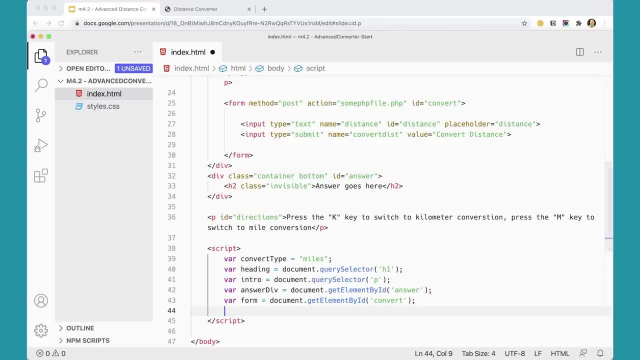 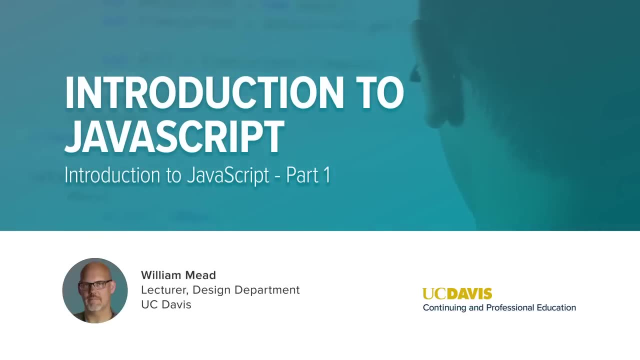 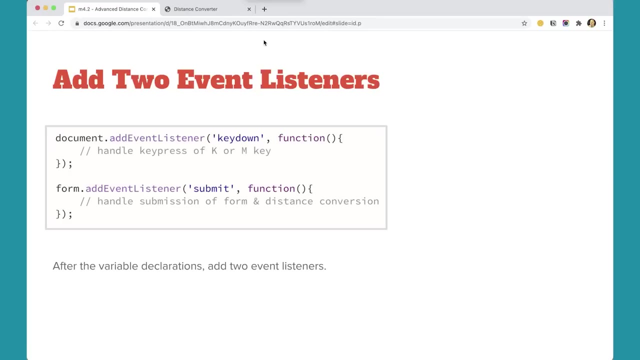 to continue the script, so we'll pick that up in the next video. okay, we. next, we need to add two event listeners. one is going to handle key down, so when we handle the k or the press of the k key or the m key, and the other one is going to handle 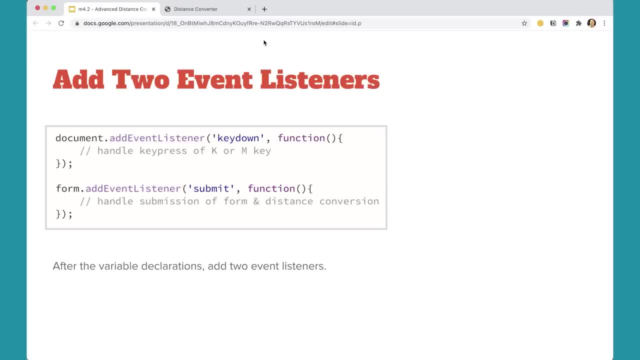 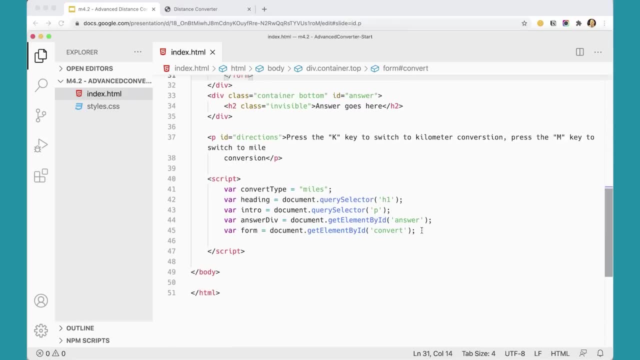 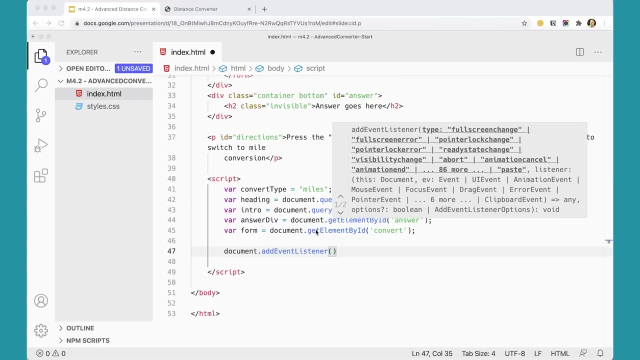 the the submission of the form. so let's add these two event listeners before we do anything else. come over here to my code. down here in my script I'm going to have document dot- add event listener and the event I'm listening for is a key down. 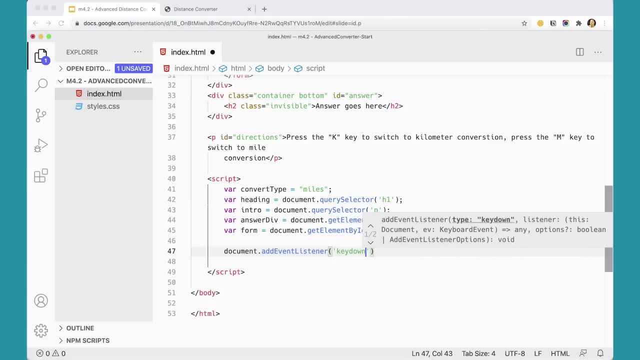 event key down and then I'm going to run a function and everything for that event listener will go between those curly braces. so that's one, and then we need to deal with the submission of the form. we already have a variable that's going and getting that. 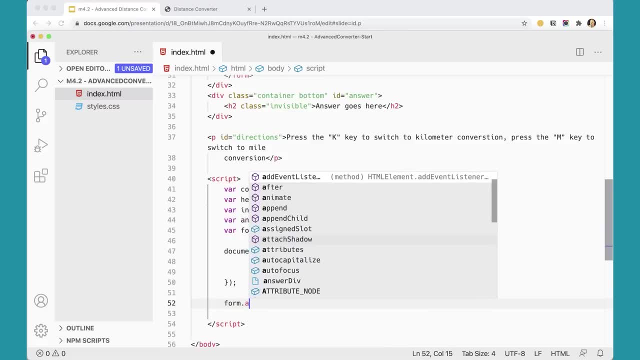 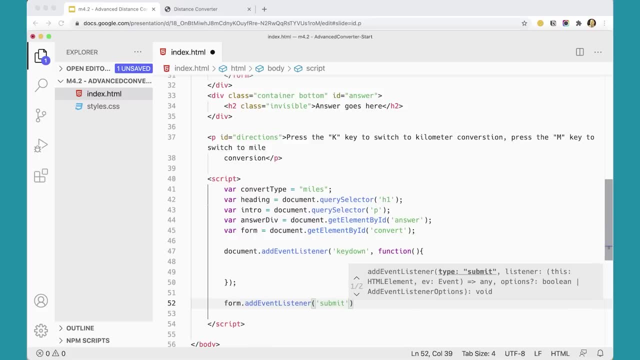 form by id so I can just do form dot, add event listener. and again we want to do submit. when the form is submitted, we want to run the function it's going to run and do all the fancy stuff. so that is going to happen in there. all right, great. 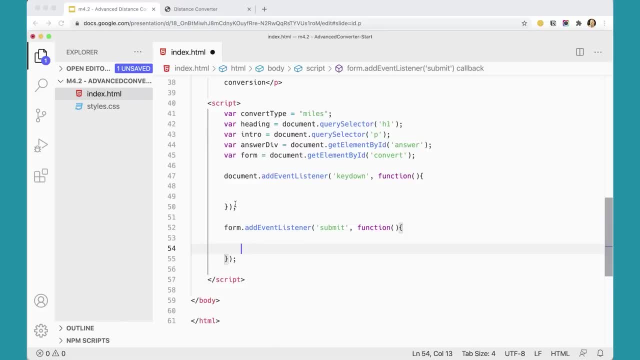 so we've got our two event listeners and we're ready to get started with this and we'll work on the key down event listener first. to do that, we're going to pass in the event object here and before we had used event dot which to figure out which. 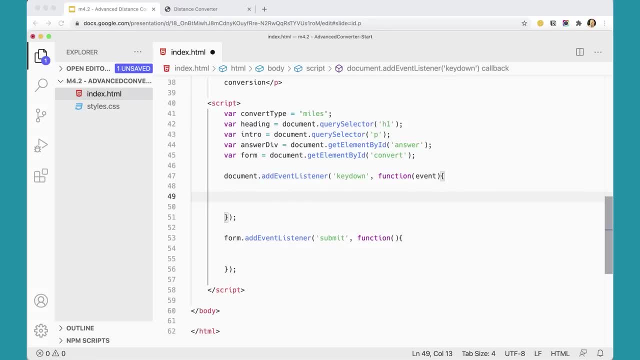 key was pressed, but event dot, which is now deprecated and really what they want us to be using over at dmdn is event dot code. let's assign that to a variable bar key equals event dot code and then I'm just going to alert out key. 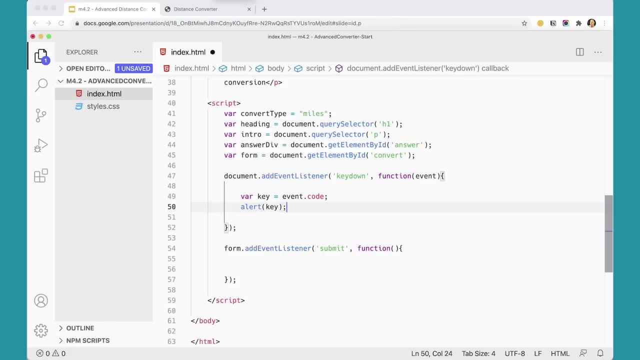 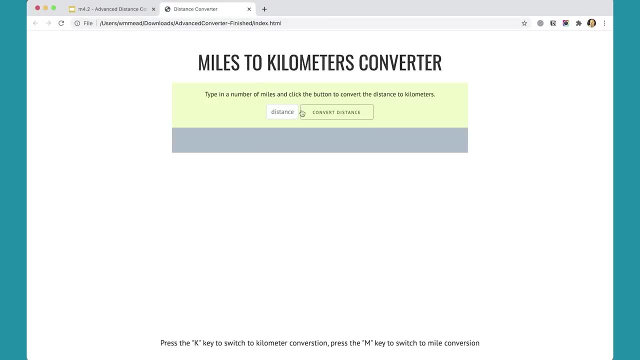 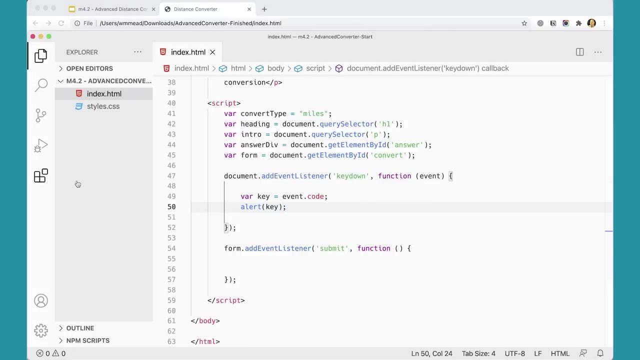 to see what I get. all right, great, let's go over here and test this. if I refresh and I press the m key, I'm not getting anything. did I do something wrong? inspect: I don't have an error alert. key event listener document. that should be right. 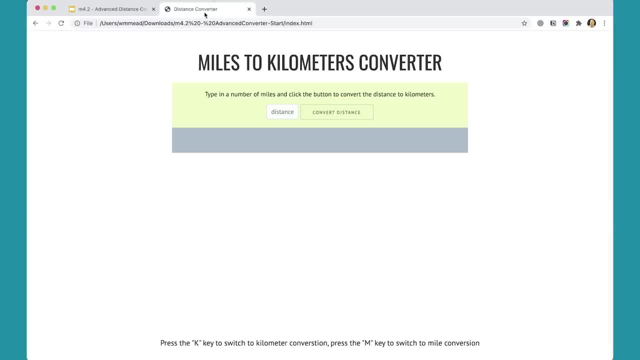 no, I did that right. I was just on the wrong file. make sure you have the right file loaded. that's always a good idea. make sure you're working with the correct file. that happens sometimes, but let's try this again. I press the m. I get key m. 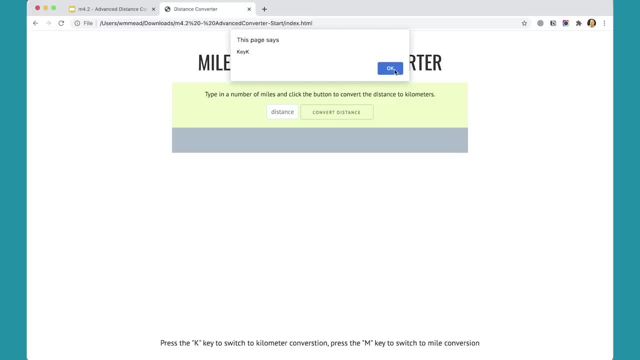 if I press the k, I get key k. so this is the new method that they want you to use. that's not deprecated for grabbing keys. instead of giving you a number, it gives you actually a key within the letter than the actual letter that you're pressing. 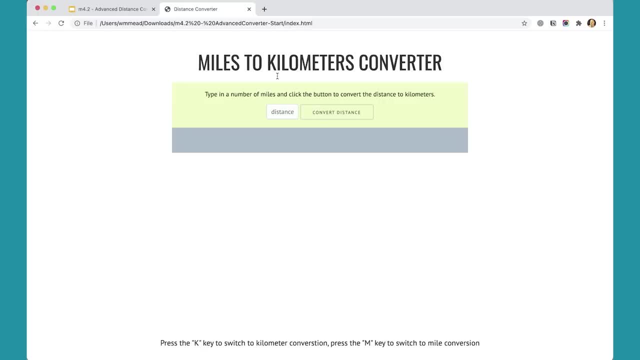 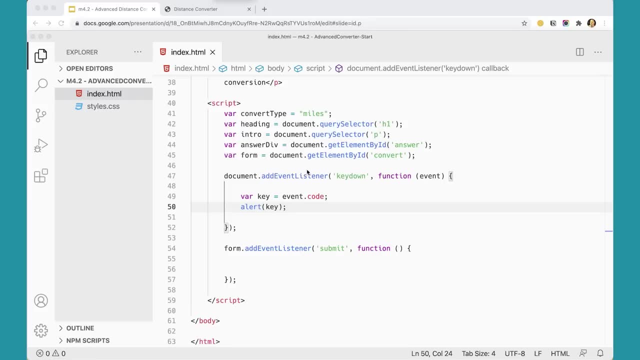 so that's great, that's super useful. so we know how to actually capture those keys and know which one has been pressed from here. writing the if statement is fairly simple. now that we know what to expect, we can say if key key is the same as you can even do triple equals if you wanted to. 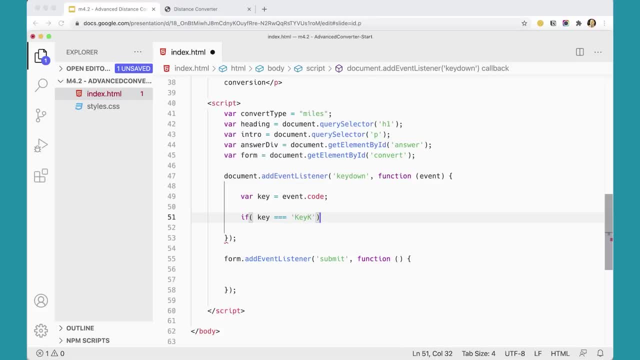 key k, we're going to do one thing else. if key is the same as key m, we're going to do something else. and what are we going to do in here? we're going to do some things, like: first, we're going to change the header. the heading. 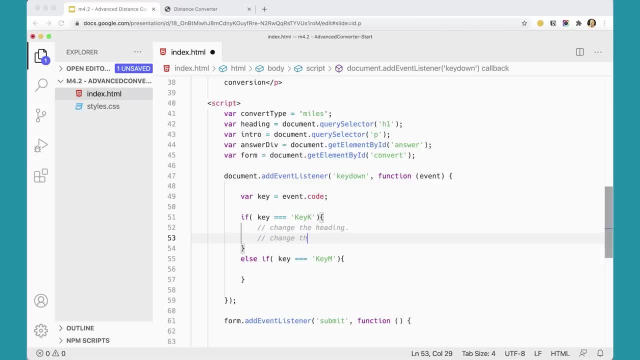 we're going to change the intro paragraph. we need to do that and also we need to change the value of the convert type variable. so we're going to change this variable from miles to kilometers if you press the k key, and then we're going to turn it back. 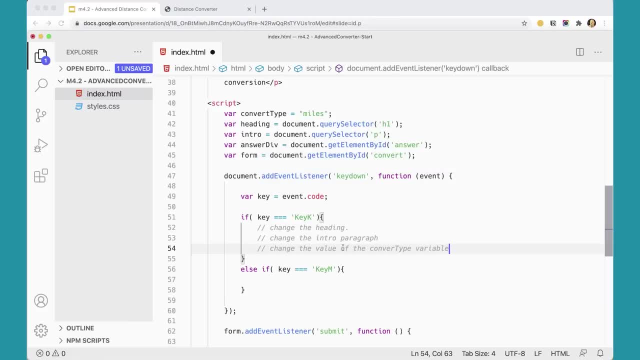 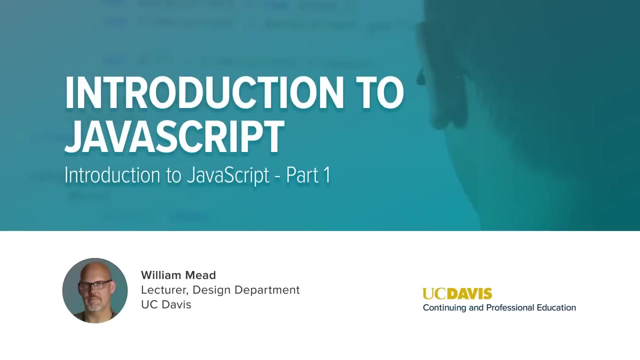 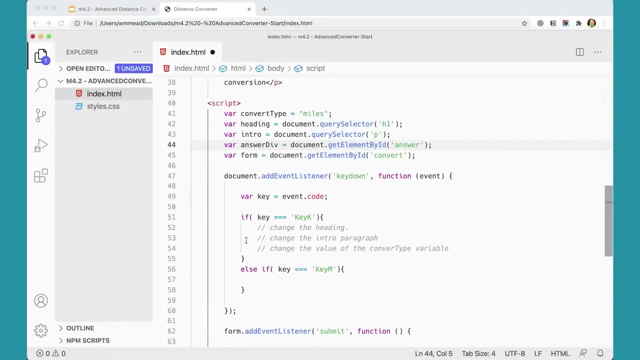 to miles if you press that one. so those are three things that we need to do in each of these. uh, if we, as we go forward here with this, this function, so we'll handle that in the next video. okay, so now we're going to put this in here, and first i'm going to do: 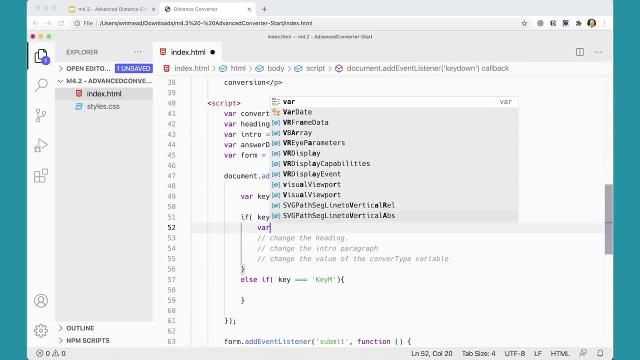 i'm going to actually do it the other way around. i'm going to have var where i'm going to set convert type. we already have it defined up there, so we don't use var. convert type equals kilometers, so that's going to get set to kilometers. 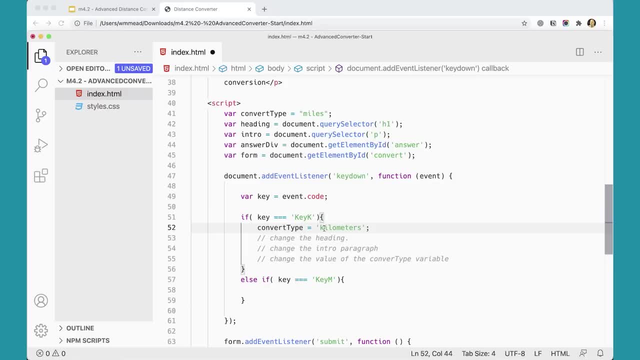 as a value as opposed to miles. you could just use k and m in there if you wanted to keep it short, and that's fine. and then i'm going to change the heading in here next. like that heading dot inner html. equals kilometers to miles converter. so that's. 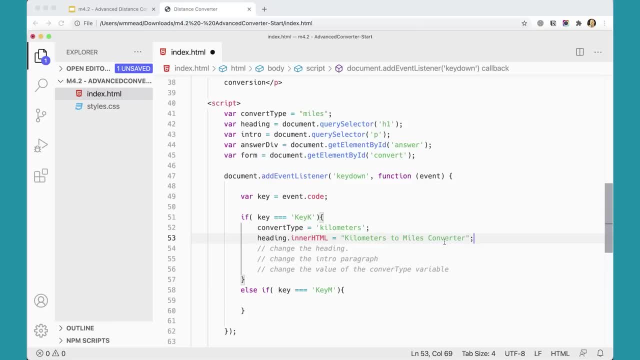 going to change that heading up at the top of the page and then the third thing i want to do is just change the intro paragraph. so let's do that next. so that's this variable here, intro. so i can very easily just type intro if i could spell it right: dot. 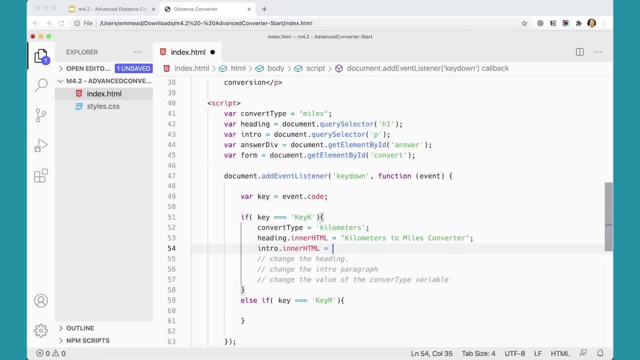 inner html equals, and then i'm just going to paste this in. but you're going to have to type it. type in a number of kilometers and click the button to convert the distance to miles. there we go. so we've got all of these set in here. 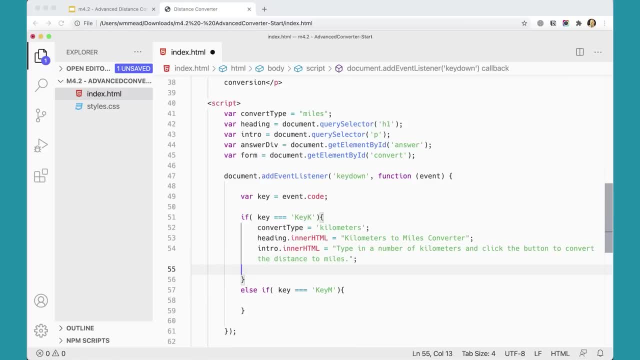 that's great, and really what we need to do is put the same thing down below. i'm just going to copy it and paste it, but instead of kilometers it's going to be miles, and then over here we're going to say miles to kilometers converter, and then 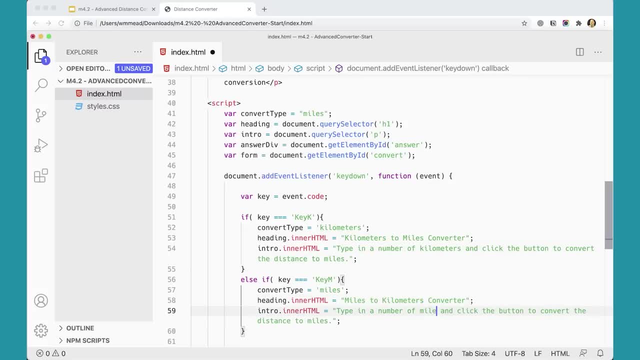 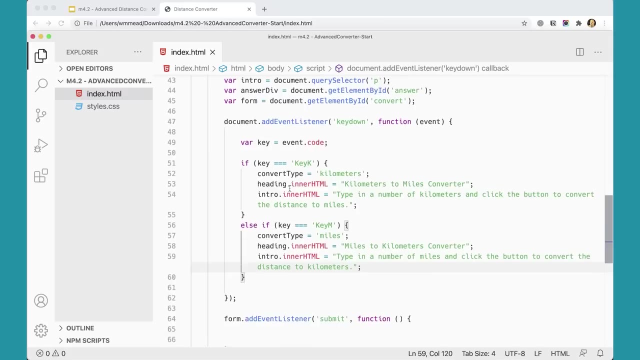 type the number of miles and click the button to convert the distance to kilometers. that's nice and easy, great, so that should be working. in terms of which key i've pressed here and how that's going to work, and if i come over and test this, you should. 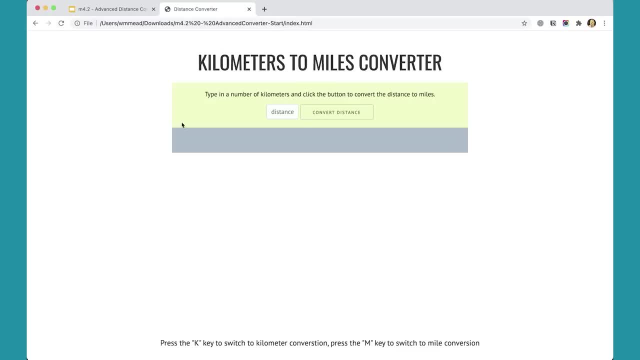 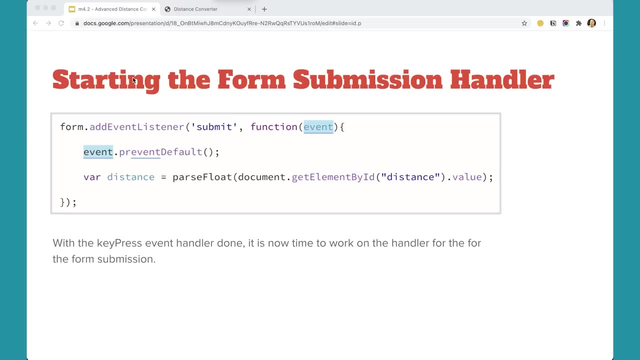 see, if i press the k key, it switches to kilometers, to miles. this statement changes, and if i press the m key, it switches back. so that's working great, so far, excellent. now we can start the second part of the script, which is the form submission handler and 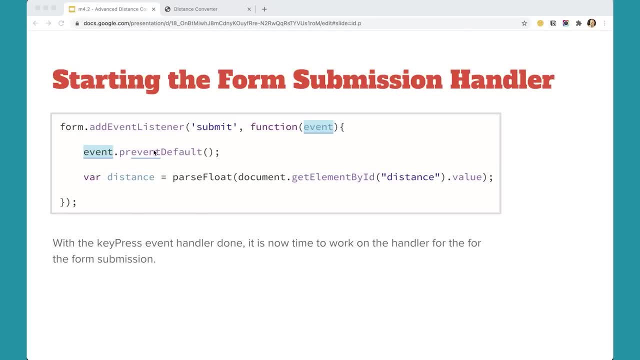 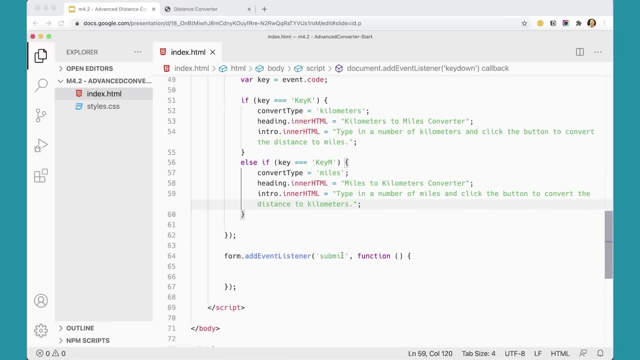 we can pass in the event and once again, do event prevent default to keep that from, keep that form from being submitted, actually submitted. so we're going to pass in our event object here and down here again, do event dot prevent default? great, and then we want to do the same thing. 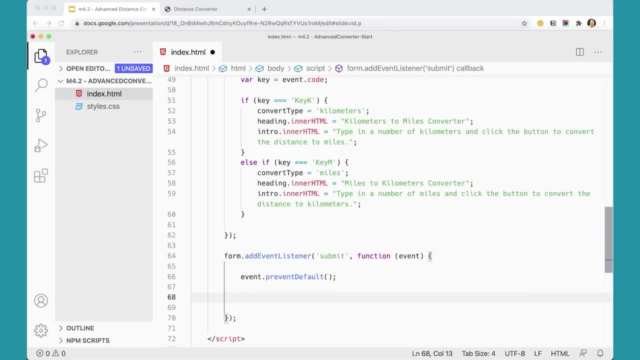 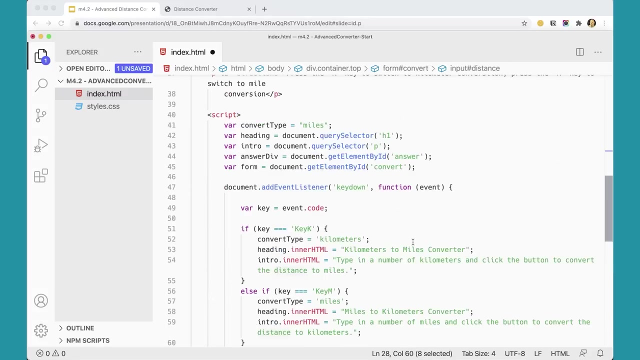 we did before and get our variable out of there. distance bar. distance equals document dot. get element by id and we're going into our form and getting the uh up here in our form. we're getting this, this distance id, here. so get element by id. distance dot value. 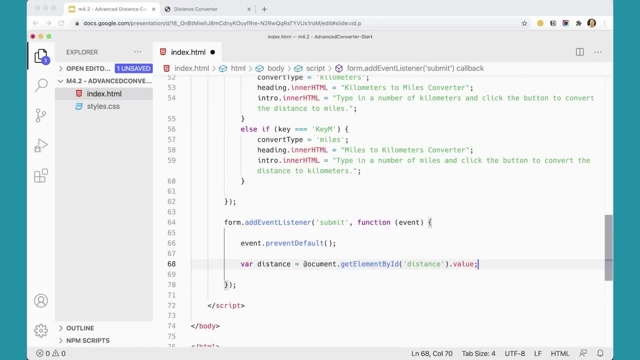 like that. but just as we did before, we want to put parse float in front of this parse float parenthesis and then close the parenthesis at the end after value there. so that will actually take that and put that in there, just like we did before. also same as before. 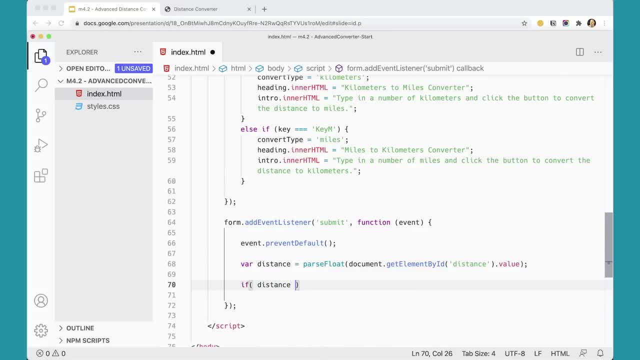 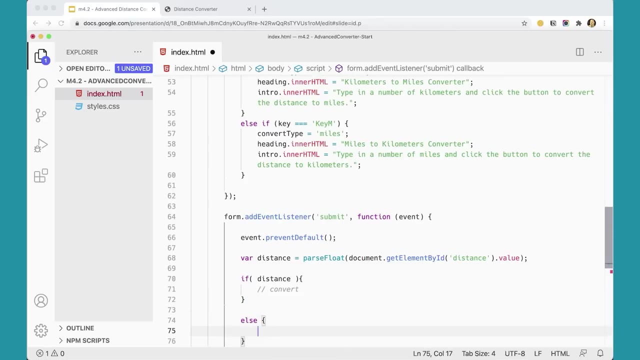 we're going to say: if distance, if that's really a number, then we're going to do something here, right? otherwise we're going to do something down here else and really what we want is just to set that answer dot inner html equal to h2. whoops. 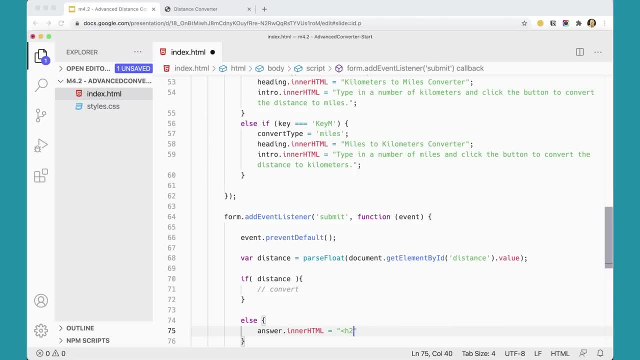 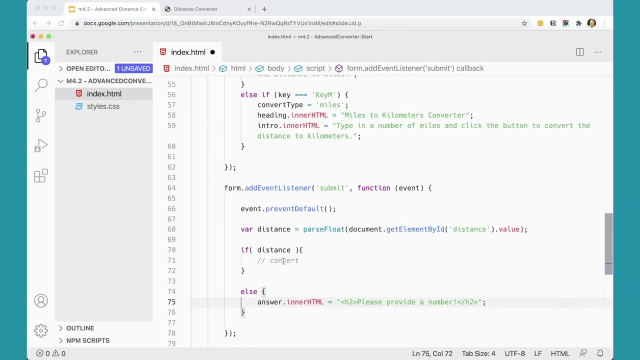 whoops, whoops, whoops, whoops. h2. and in there i'm going to just say: please provide a number, something like that. that's fine, so that will handle the error down there. if somebody doesn't put in a number in here, what we're going to do is we're 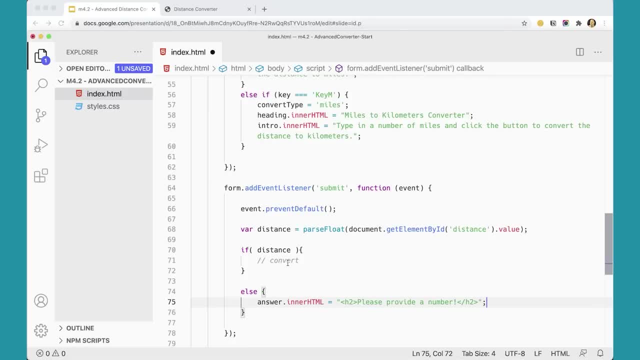 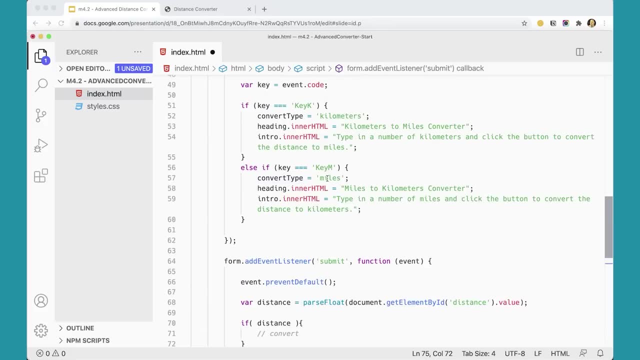 this is where we're going to do something different and see if you can think about what we need to do. we need to need to check to see what the value of this variable convert type is, because it's either set to miles or kilometers, And this is one reason why we set this variable. 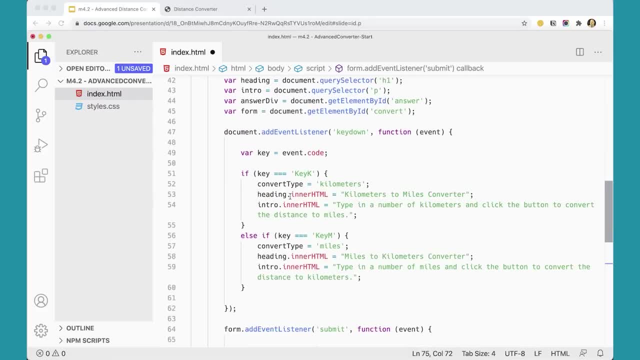 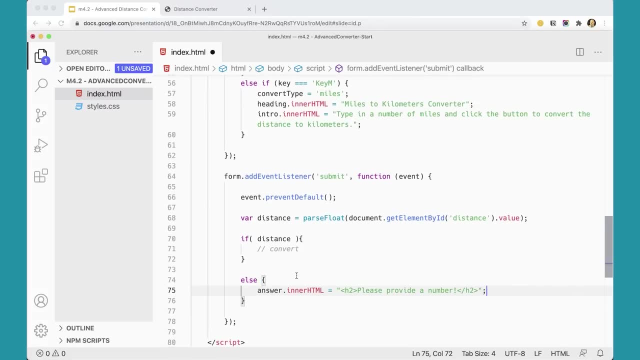 we initialize this variable out here in the global scope, so we would have access to it down here as well, inside this event listener function here. So we want to be able to have access to that variable there. We need to see what it is, Because if it's one, we're going to do one type of conversion. 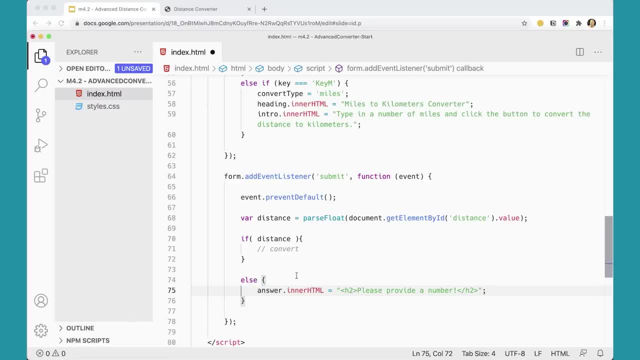 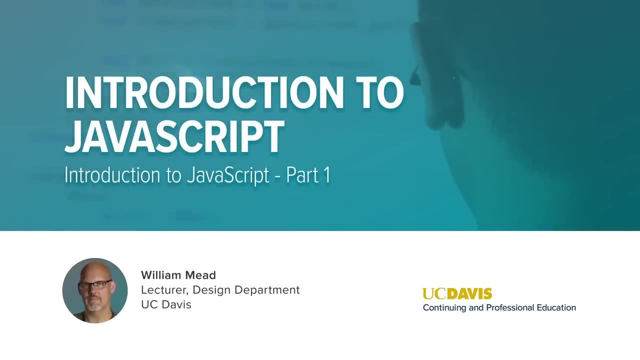 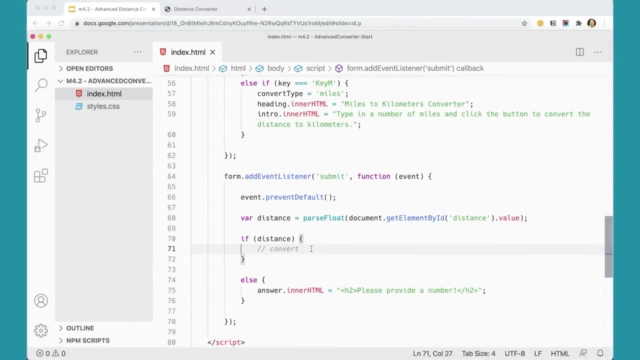 If it's the other, we're going to do another type of conversion And we'll look at that next. OK, so now we need to actually do the conversion here, and based on which value this variable has here: convert type. So to convert miles to kilometers, the ratio is this: 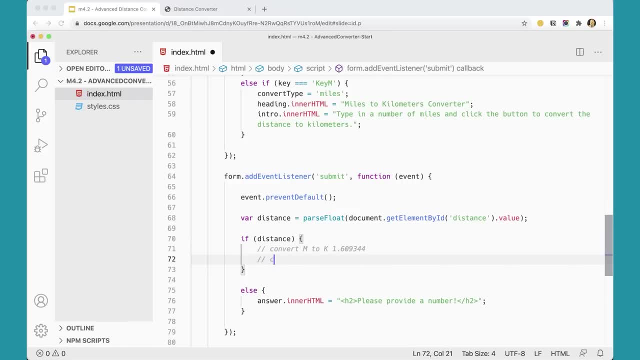 And to convert K to m, the ratio. is this OK? so see if you can figure out what we need to do inside this if statement to handle both the conversions. See if you can get it on your own. Pause this video and see if you can write the if statement. 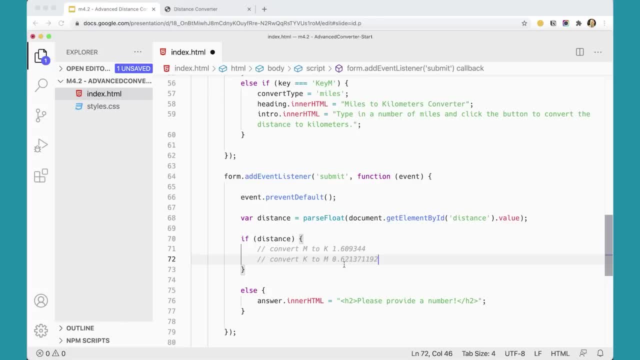 you need in order to do this, using these two values for numbers here. Hopefully you got something like this: If convert type is the same as miles, we're going to convert that there, else we'll convert the other one. OK, OK. 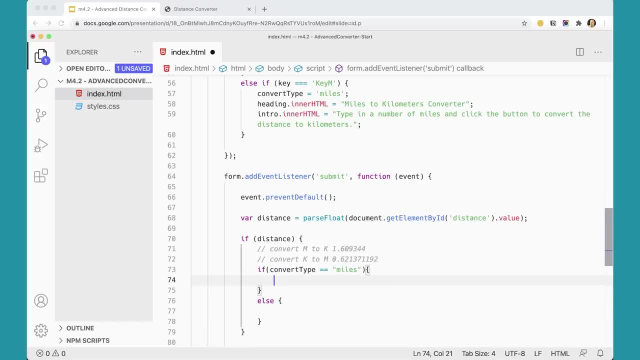 OK, OK. So if it's the same as miles, we're going to take distance. We're going to have variable var converted something like that equals distance times this number here, And then we're going to put parentheses around that. 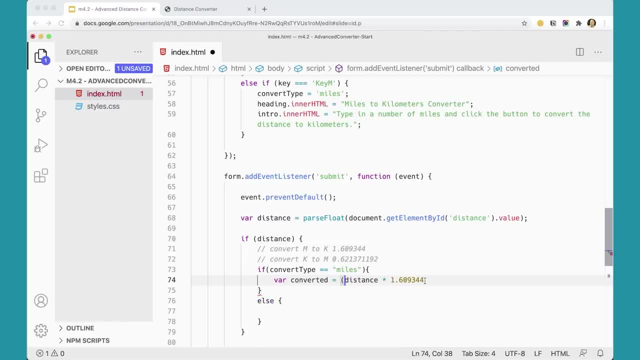 Right Now we can put parentheses around that And then do to fixed to give us three decimal places. So that's what happens if we're converting to miles Whereas down here in the else converting to miles, converted is going to be set to this value. 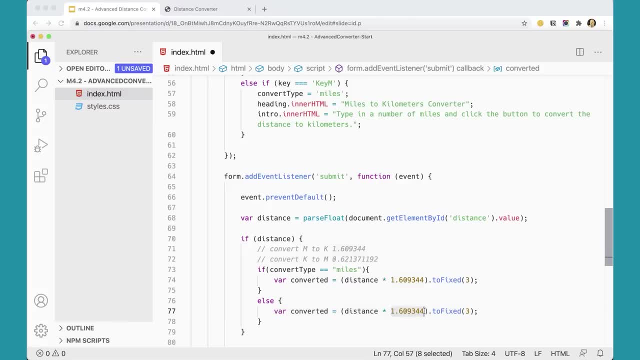 And then we can just set the answer: div right. AnswerinnerHTML equals. And we're going to use our tick marks And we're going to say: enterHTML equals. And we're going to use our tick marks And we're going to say: enterHTML equals. 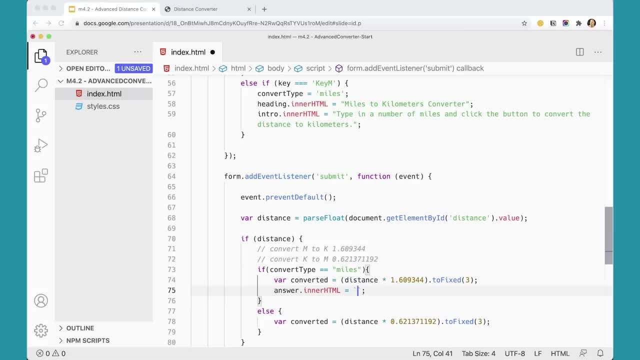 x miles converts to y kilometers, but x is now going to be not x, it's going to be dollar sign curly braces, oops, curly braces. and in there i'm going to put distance converts to dollar sign curly braces. converted. there we go and down here it's going to be the same thing. 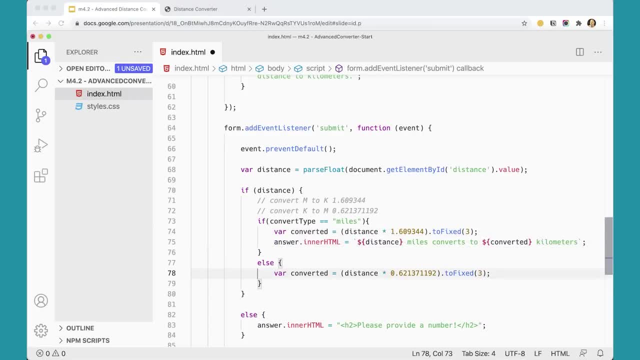 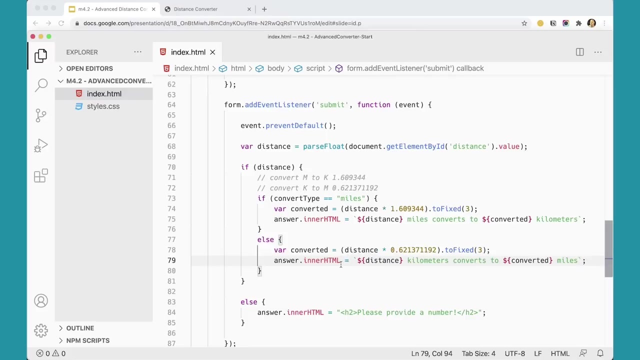 answer. copy that, stick that down here. except instead of miles that's going to say kilometers converts to miles. save that, there we go. so now we're able to convert both miles and kilometers and put the correct answer. yet if somebody enters in something that's not a number, 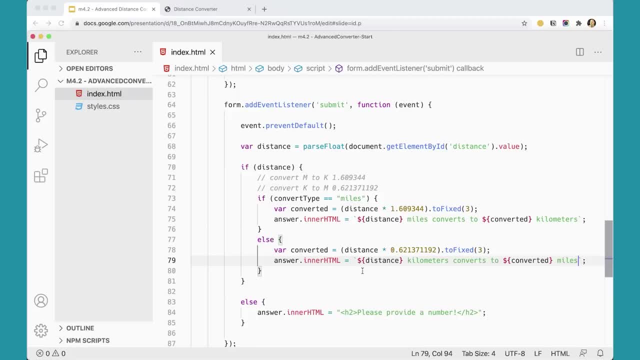 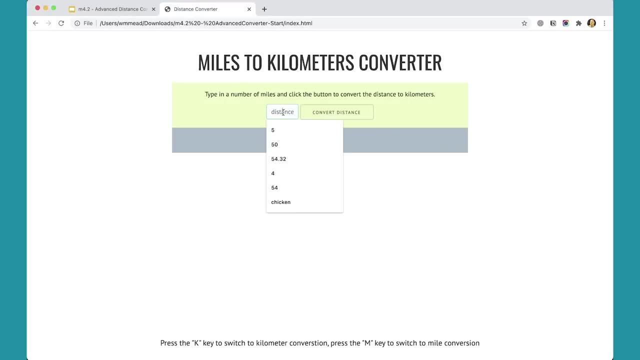 that will still be handled and that should work. let's test it and see. refresh miles to kilometers. if i put in one mile, that converts to 1.609 kilometers. that's correct. if i press my k key kilometers to miles convert and i get 0.61. 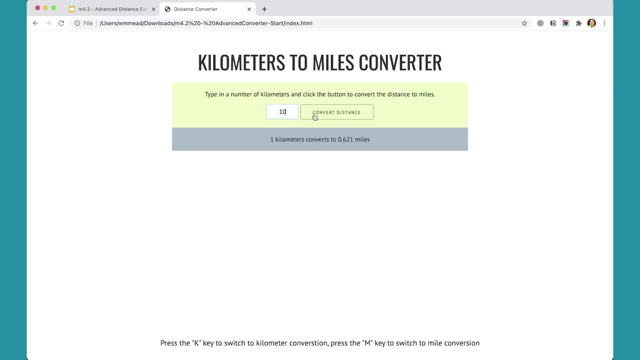 miles, and that's correct. do 10 and test it and you'll see that you'll get the correct answer and you can see that that's working. so there we go. we have a working distance converter for a more advanced, a more advanced distance converter that will allow us to switch between: 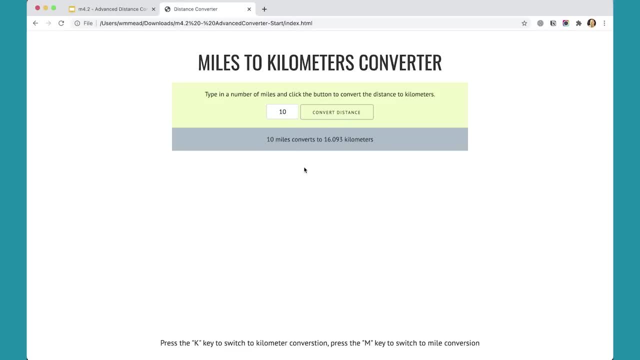 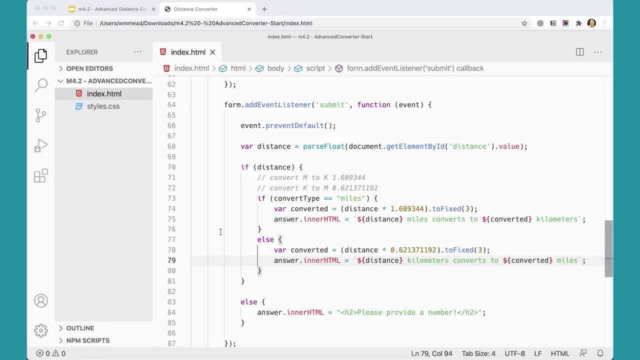 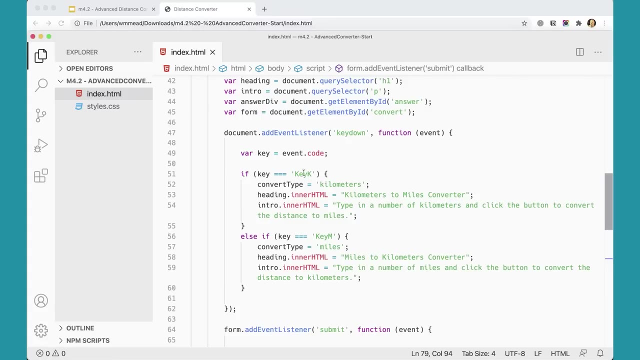 uh, miles and kilometers for our converting and over here in our script. the important thing to recognize here is that we're using a variable up here at the top, convert type, and we're adjusting the value of that variable to the value of the value of that variable here based on the key that's pressed. 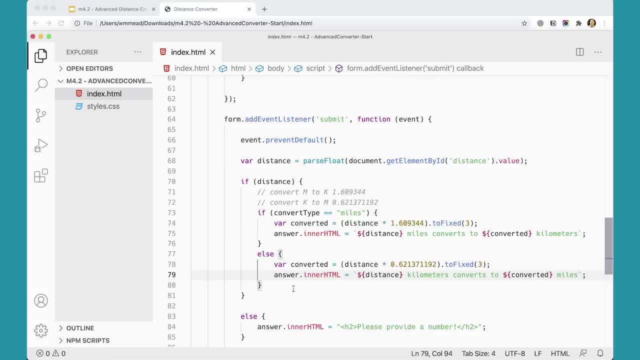 and then based on the value of that variable, in this function down here where we're adjusting which one of these we're going to be using based on what the value of that variable is. now, this is where we're starting to get into some scope and some um, a little. it's. it's a little bit more. 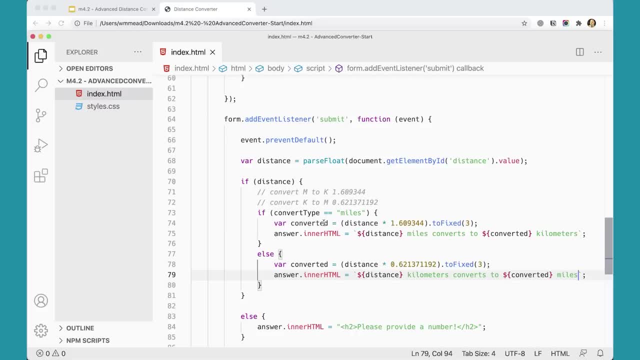 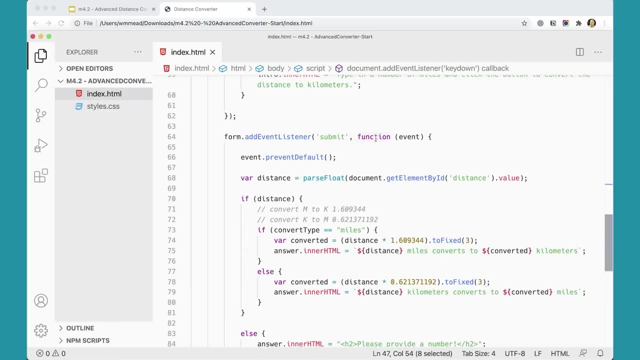 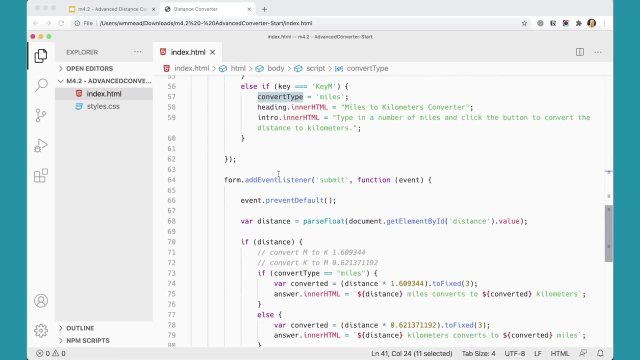 complex, because we're looking at a value that you need to get set in this function here and then access it in that function there, and we're doing that by defining the value up here. so that's pretty cool. so the last thing you should do with this: 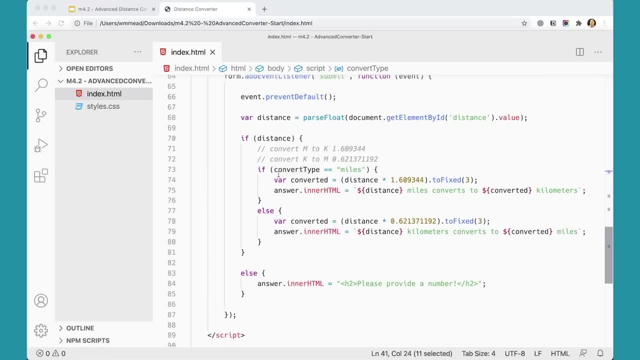 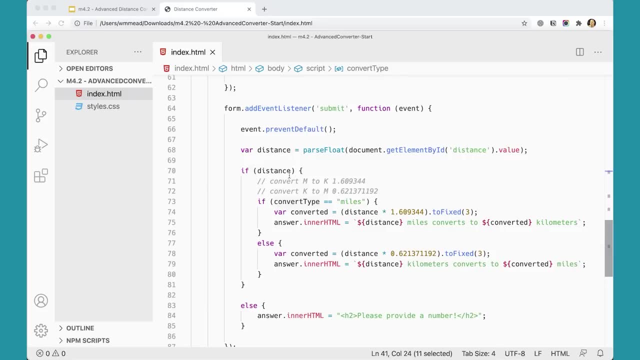 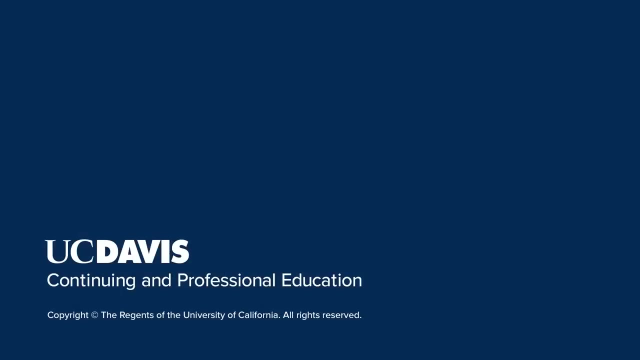 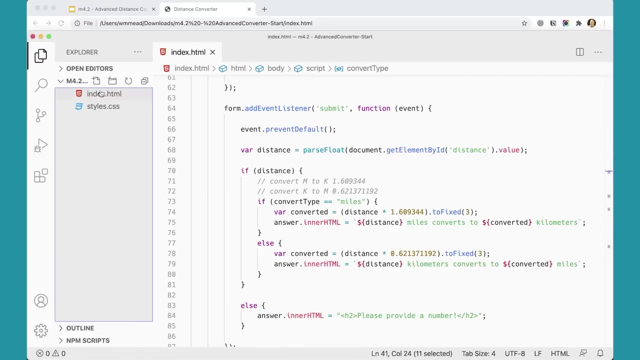 is: put it all into a script file at the top of, and and link it at the top of the page instead of having it here in the bottom, and use all your best practices for that. you may not need to watch this video right now, but because you should know how to do this already. 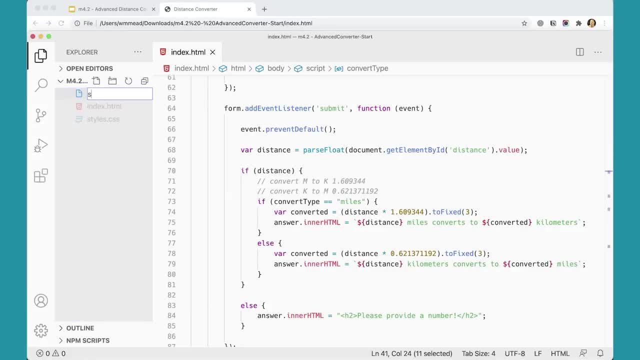 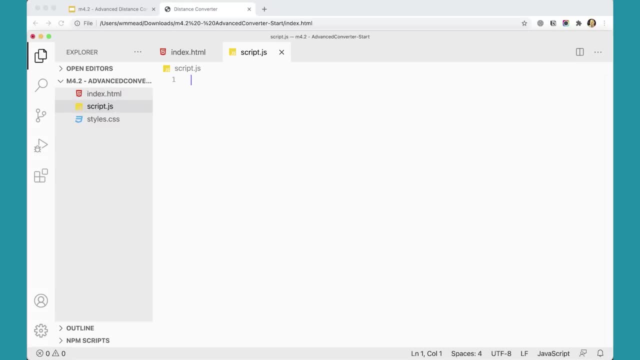 but i'm going to do it anyway. i'm going to create a new file here called scriptjs, and really you can name the file whatever you want, and on this file i'm going to add my um, my function here, my function that will run automatically. function with its parentheses and its curly braces. 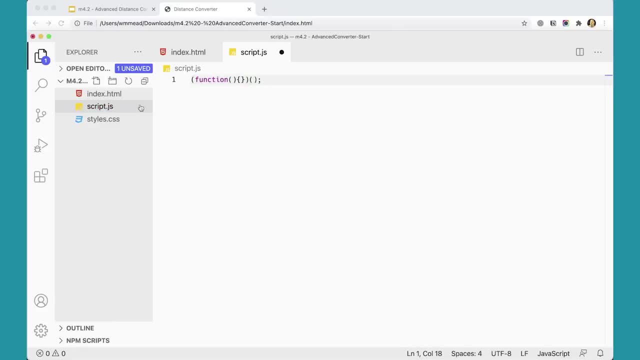 and an extra set of parentheses at the end. this is my automatically invoked function here. and then everything's going to go inside the curly braces, and down here i'm going to add: use strict that directive to make sure i don't have any variables being defined in the wrong place. and then i'm going to come in here and 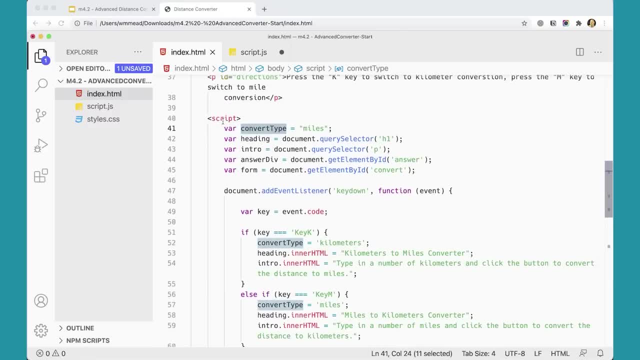 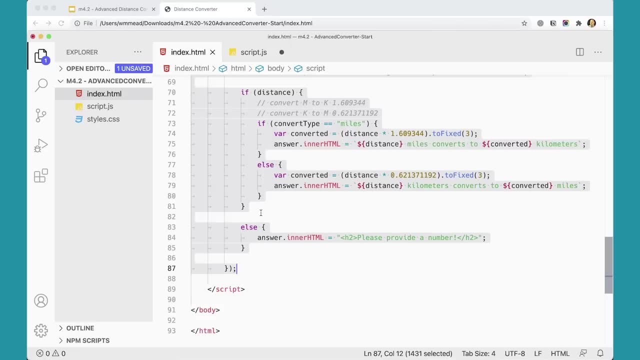 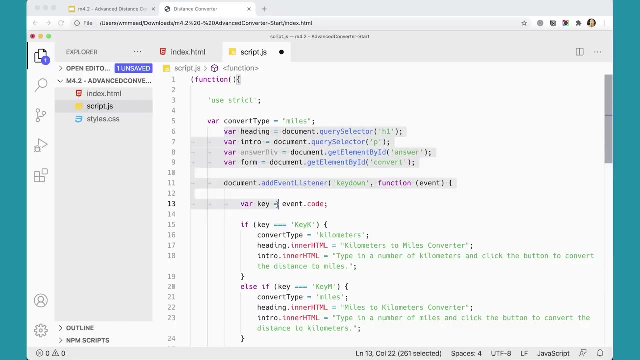 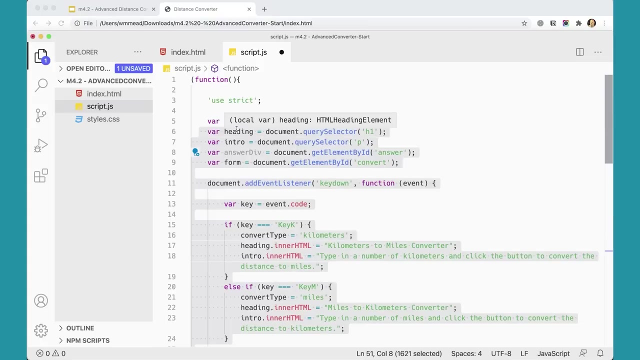 just copy all of this script, the whole thing, all the way from the top, all the way down to the bottom. i'm going to paste it over here, i'm just going to paste it right in there, like that. i need to tab it back. one shift tab. there we go. now for this one. it's more important to do this than we. 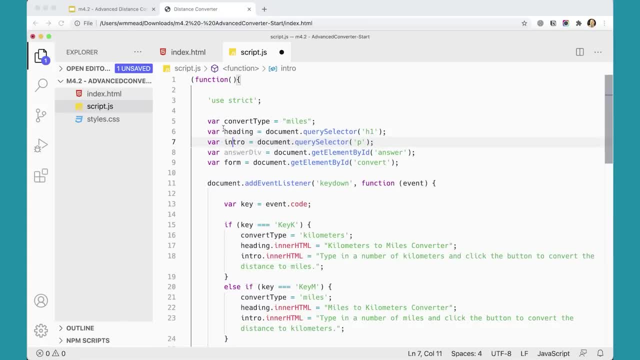 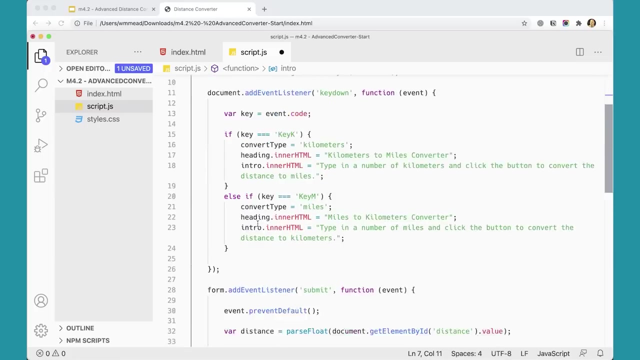 did for the previous script, partially because there's more code going on here, but also also because we actually have some globally defined variables here and it's possible that you um don't want them, that you you want these to not get um get used in the wrong place down there. answer: div: that's gray. did i do the wrong? 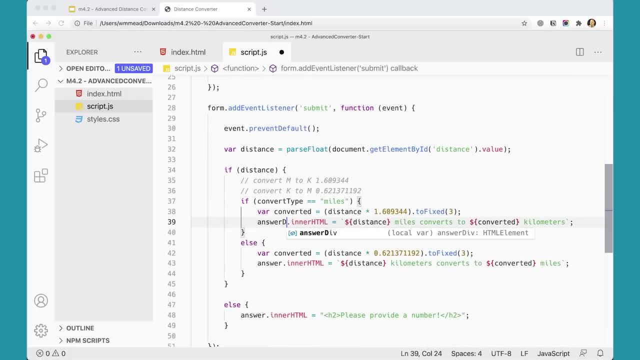 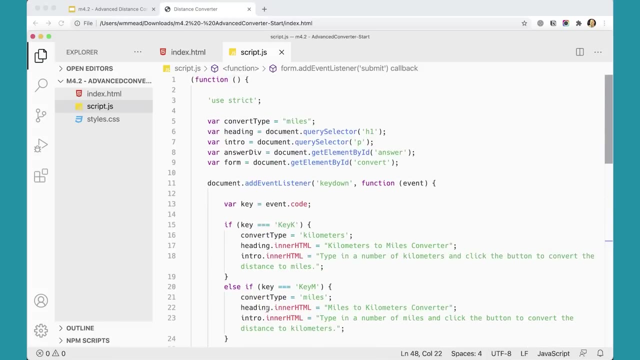 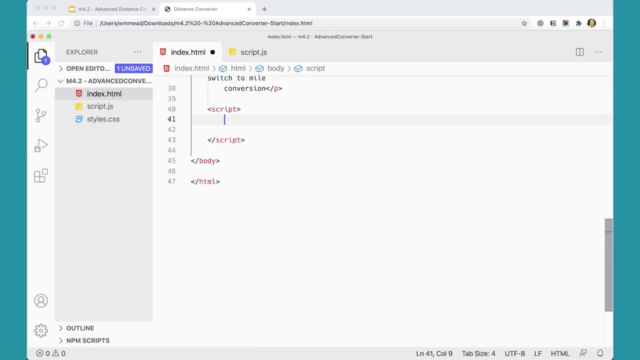 thing down here i did should be answered: dip answer, dip answer, dip. there we go make sure that matches. okay, so, um, so that's putting that. that should put that into the right place there. okay, great, so over here in our file. here we can get rid of this stuff. 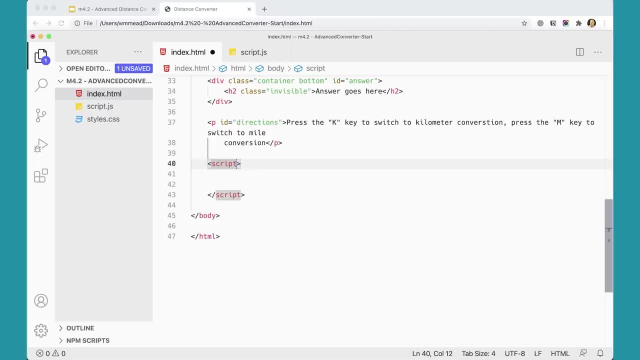 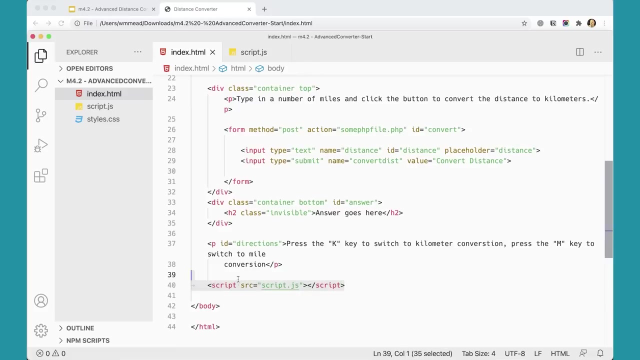 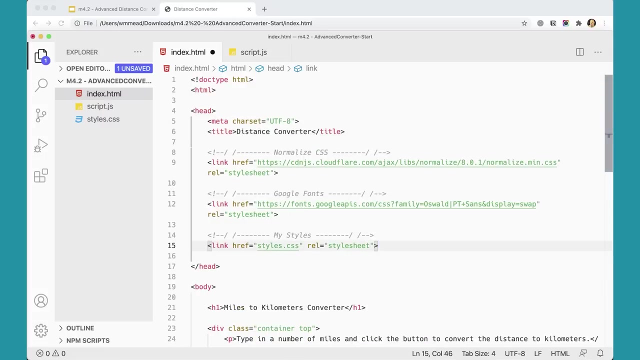 and instead we can link to src equals scriptjs. there we go and there we have it, so that should work great. now we could move this up to the top of the file here, and then we can try to convert it and make sure it can be passed to our. 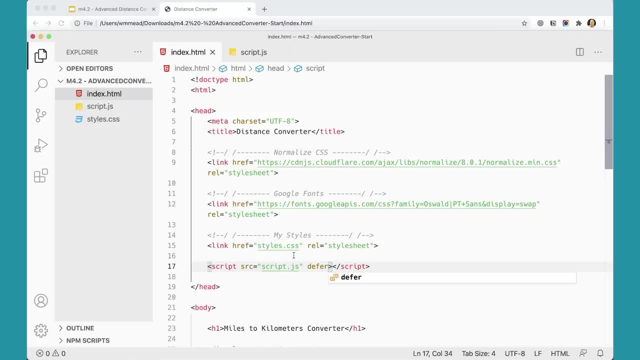 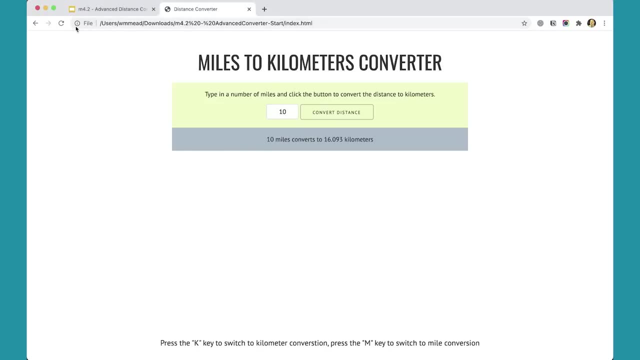 command prompt defer. there we go, and that should all work just as well. so if i come back here and refresh this distance, five convert, that's working. 10.10.99.03.14.27 convert- and that's working. so um, and i should be able to press miles to kilometers and do the other. 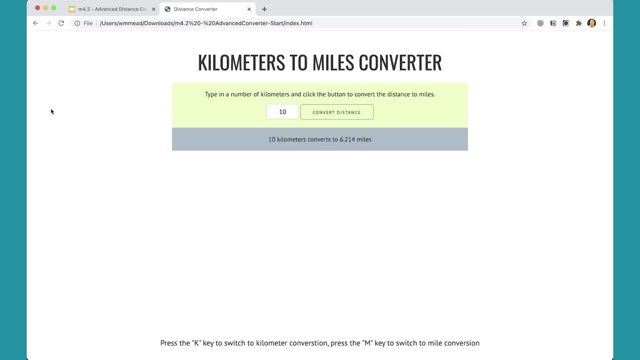 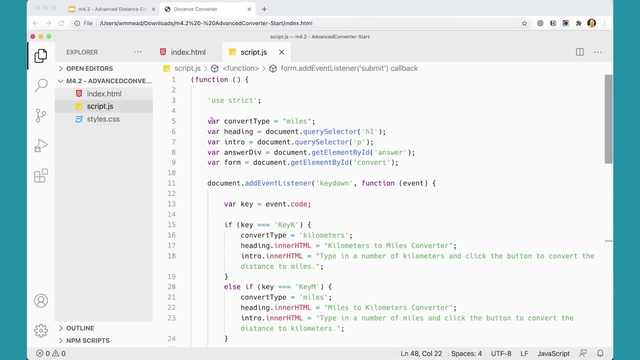 conversions as well. so that's all working perfectly fine and has been refactored a little bit so that this is all over here. oh, the one last thing i didn't do is i didn't come in now. this one needs to be let because that one's going to actually change values. this one can be const. 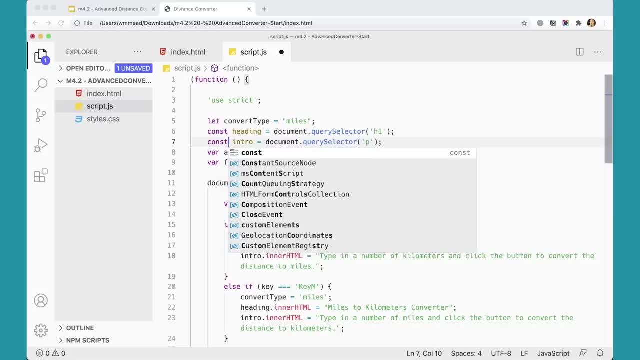 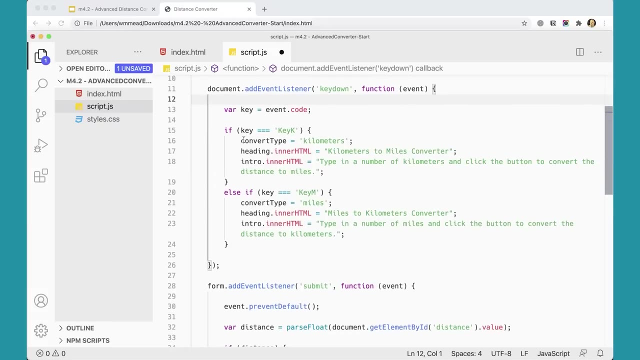 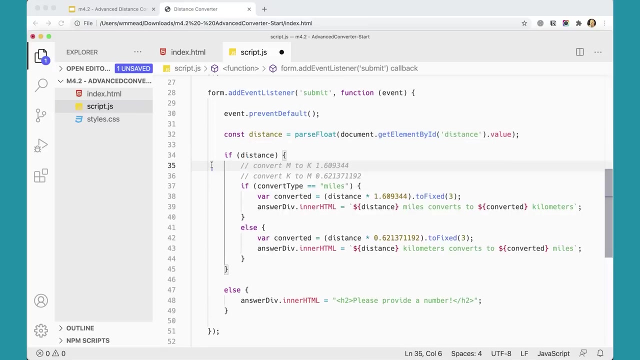 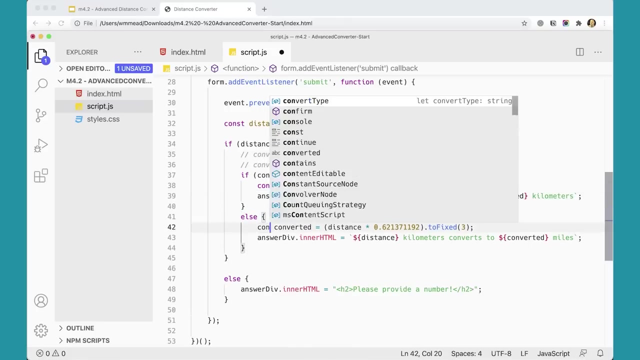 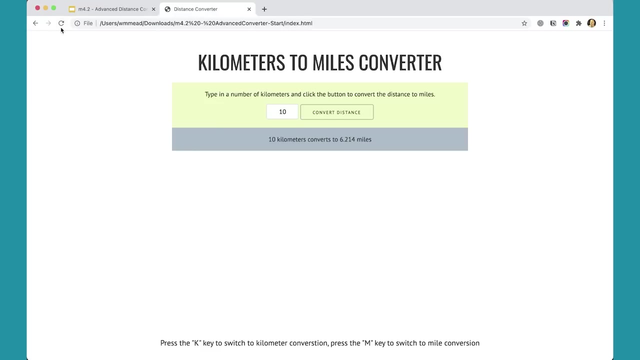 this one can be const, this one can be const, const, and then down here, const, const and const and just test it one more time. always test to make sure you didn't set the wrong thing, but it should work. five miles, press the m k key, test it again and that's working. just great, okay, great. 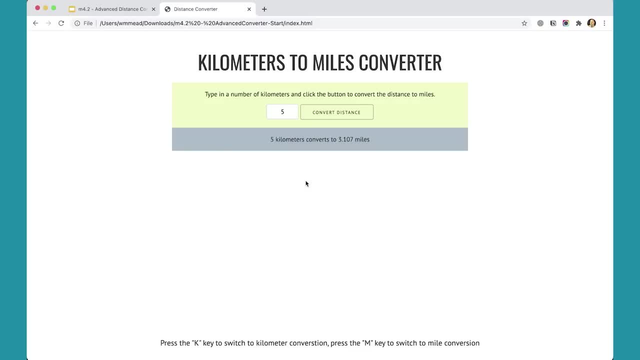 so we have a great little utility here for converting miles to kilometers and kilometers to miles. not that you needed something like this, but we have used a lot of the kinds of things that we've learned about in this course so far in terms of capturing some data from a form, being able. 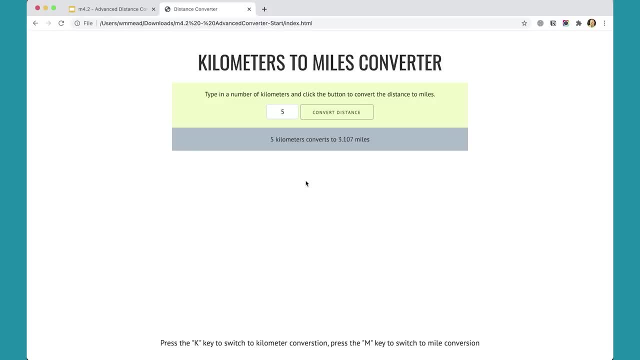 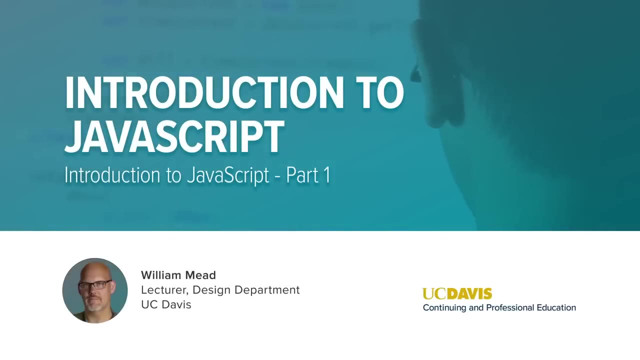 to manipulate that data and then change the dom, change the actual web page, based on what the user has done, including capturing key presses, which is pretty neat physics so common enough. just have to look into that. yeah, we've got a Java over here at our top which Kadica and 뭘 goal-asha. 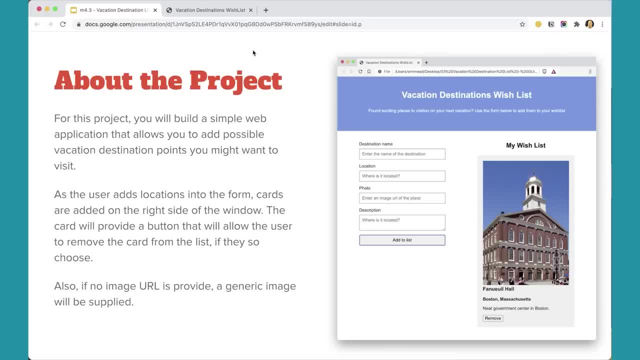 let's hit that um. so that's our overview for the basic project here. so make sure you're lights out and then you can go back and type in the prompt 안, and then after that we'll get into the API in just a second, if I recall. 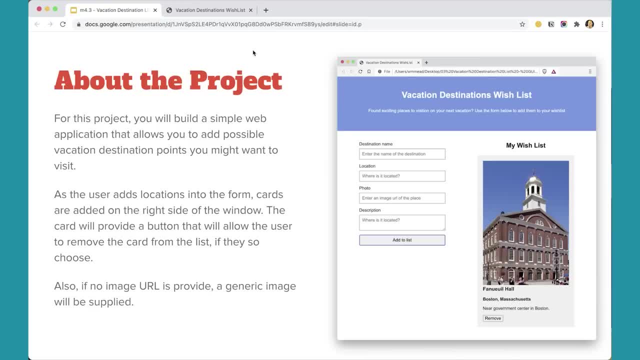 actually not like that, but we'll call it an app, for lack of a better term, if you want to think of it differently. and basically what we'll do here is we'll have a form and you can add a place that you want to go visit or see in the form and it will add it to your wish list with the picture and everything. 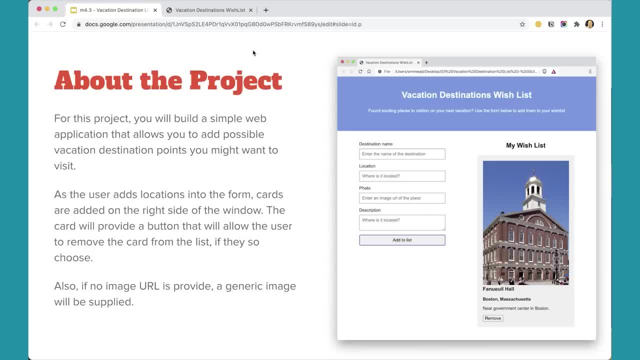 so that's pretty cool and pretty fun, but before we get there we need to build up the html and css, and in previous projects i've given you the html and css done, but with javascript, because it's such a relationship between javascript, the html and the css- the three of them together, working together. 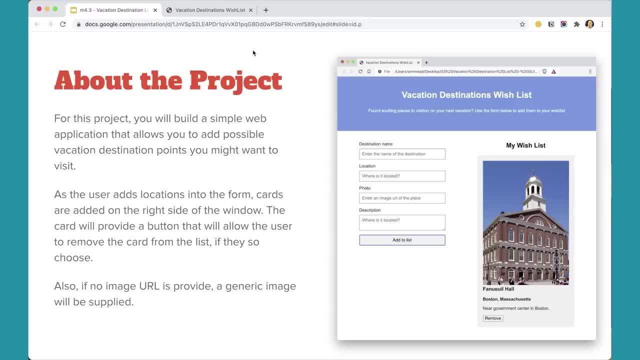 to create your interface. it's important to see how the html comes together for this project. it's not super complicated, but it's definitely more complex than the previous projects. we've done the distance converter projects, you and those kinds of things, so this is a really great capstone for the end of the first course. 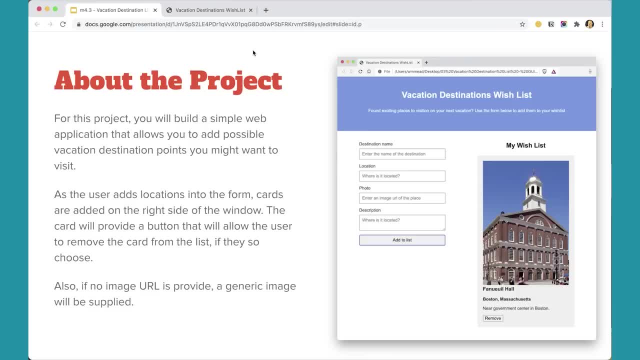 which will really bring together everything that you've learned in this course so far. and again, we've got three more courses to go after this, so you'll become an expert with javascript if you keep going. but let's start here. okay, the user's going to add some, some information to the page. 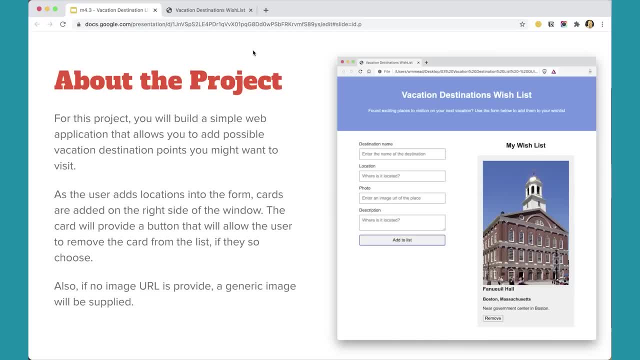 here and including a url for a picture, and then we're going to add some information to the page here and including a url for a picture, and then we're going to add some information to the page. but if no url for a picture is provided, it will put a generic image in there for them, and if we go, 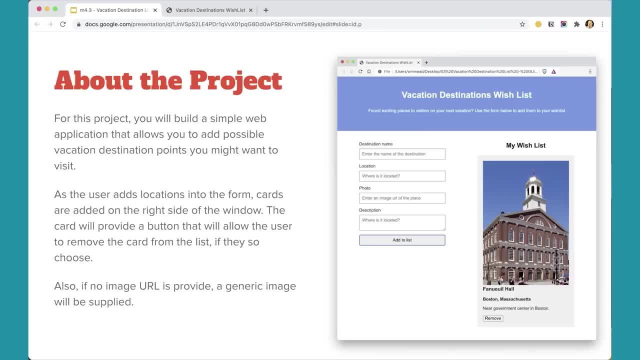 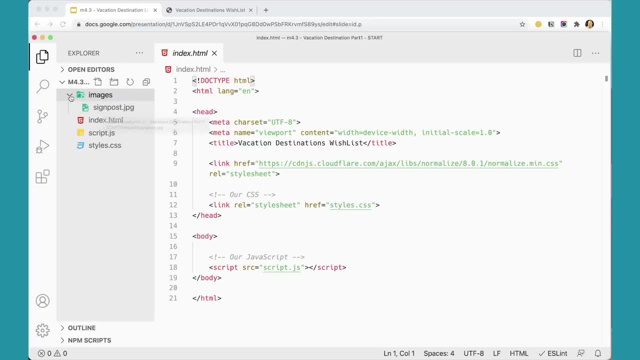 over and look at the files that we've got, the start files that you're going to start with. you'll notice that we have some images in here and i have a signpost jpeg that's going to be used as a default image there if an image is not provided by the user when they add their item to. 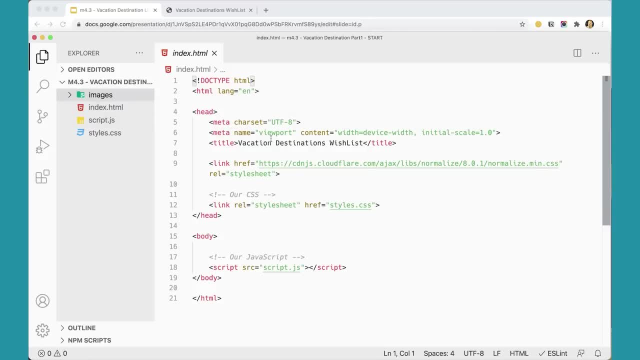 the list. other than that, the page is fairly simple. we've got a lot of information that we've got to have a lot of information that we've got to have a link to the normalized css script, which all that does is make sure that different browsers render pretty much the same way. 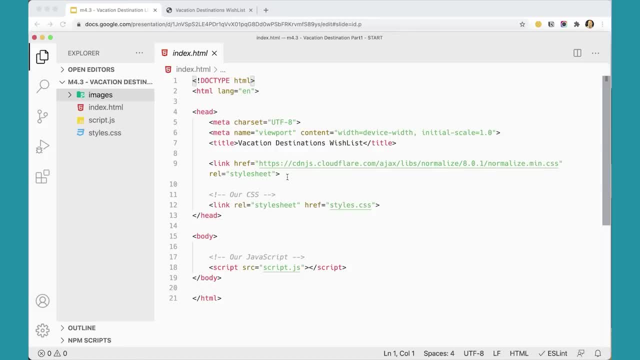 sort of normalizes the differences between different browsers and the way they render things, so that you don't end up with a different looking page in a different browser. usually it's just minor things like different spacing and stuff like that, but, um, that can be frustrating if you're a designer and you're, you want it to look a certain way and and it and it changes up. 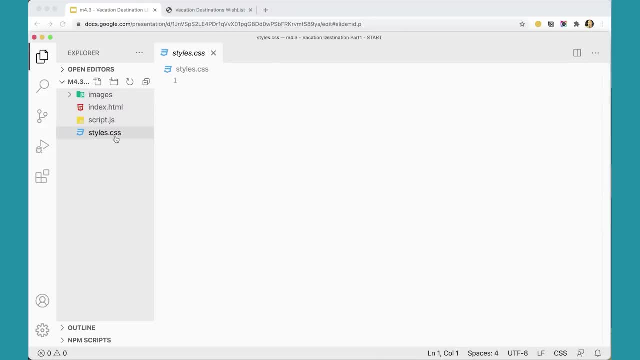 plus, if you're a designer and you want it to look a certain way, and and it changes up, we have linked a style sheet which is currently empty, um, and we'll be adding some styles in there. and then, on the body of our page, we have linked a javascript file which is also empty and in part. 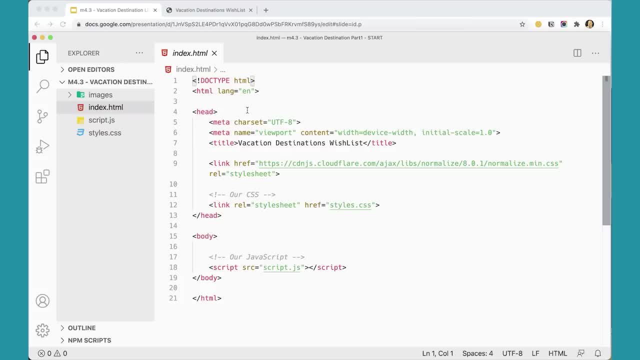 two, we'll actually be building the javascript for this project. so that's where we are. let's see where we need to go first. to get this thing started, the first thing we need to do is add a header element which will open and close, and inside the header element, i'm going to add an h1 heading and a. 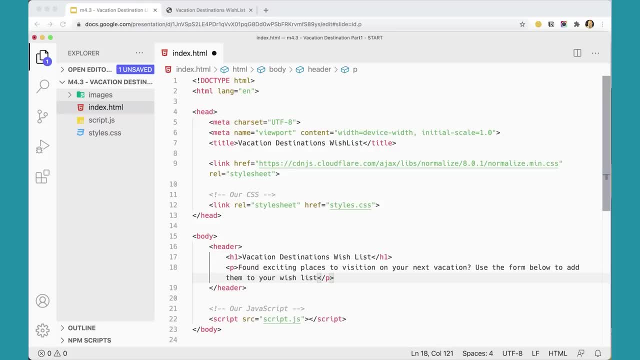 paragraph and i'm going to paste them in here. but you're going to have to type these. so the h1- vacation destinations with wish list- that's going to be our main h1 for the page- should have. your web pages should have a main heading, if at all possible: um, that google will search and index. 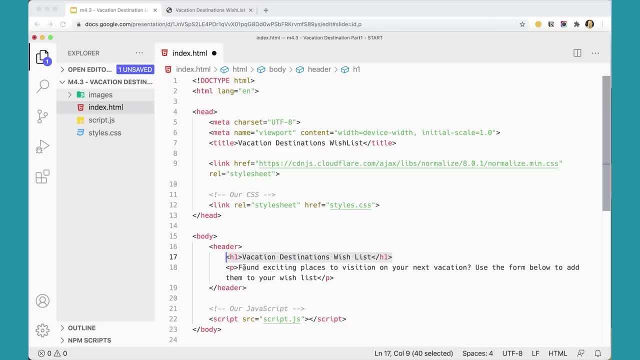 and that kind of stuff. and then i've got a follow-up paragraph: found exciting places to to visit on your next vacation. that's my english there: places to visit on your next vacation. use the form below to add them to your wish list. probably should put a period at the end of that. 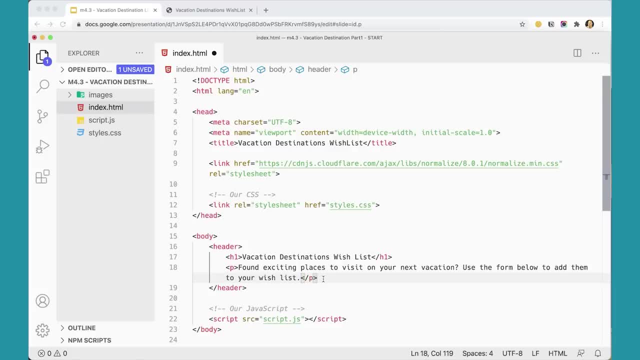 paragraph too. so there we go. so we've got kind of a place to start here and a little bit of language to get us going. once you have that done, after the header add a main element, and inside the main element we're going to add a form. 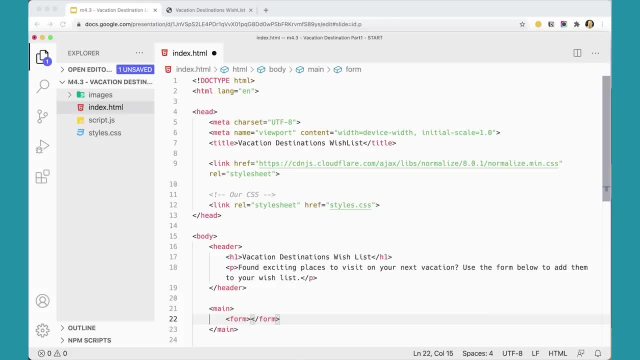 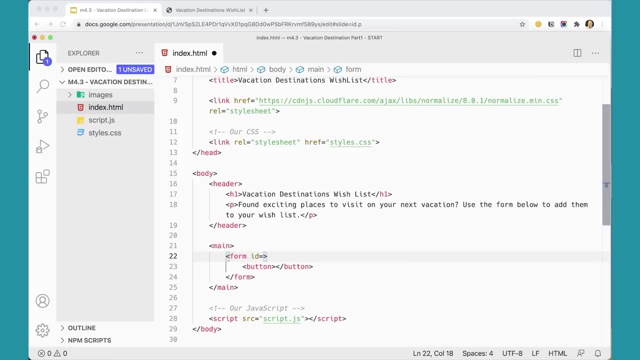 which is going to open and close, and then inside the form, we're going to add a button which is going to open and close. the form needs an id and the id that i'm going to use and you can use something different if you want, but because this one's a little bit long, but, um, but it's kind of descriptive for me, so i'm 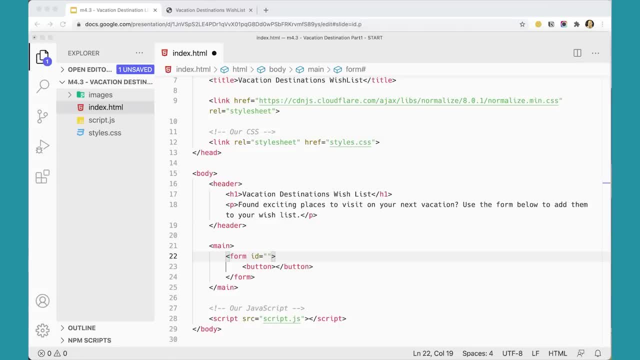 going to use this id destination underscore details form, no spaces, destination details form, and then the button is going to get a type attribute: type equals quote, submit. there we go, and then we need to add some text to the button, which is going to be: add to list, something like that, add to wish list, something like that. 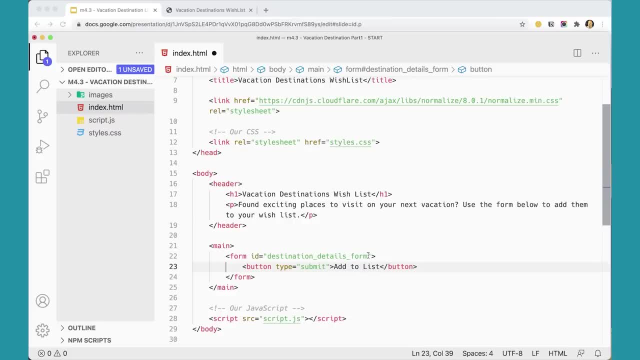 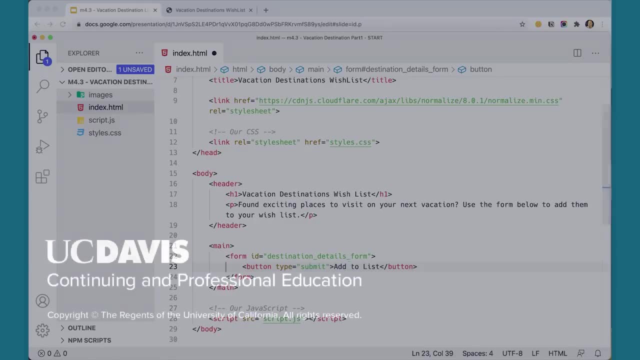 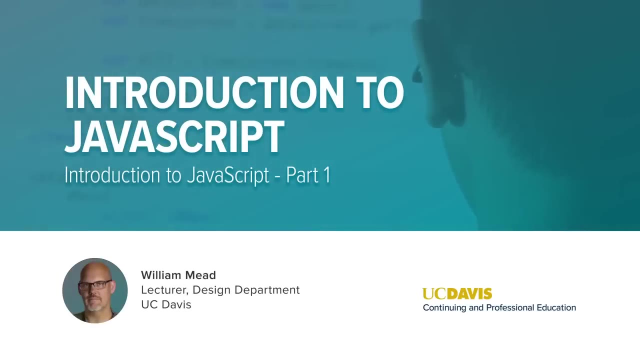 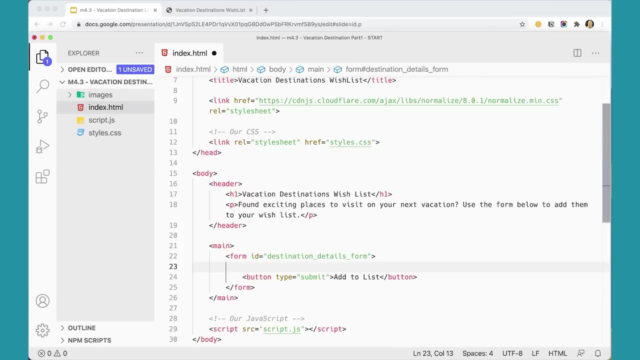 that can be the text that shows up on the button here. okay, great, we'll stop here and we will pick this up in the next video. next, we'll add two fields: one is going to hold the name of the destination and the other is going to hold the location of the destination. 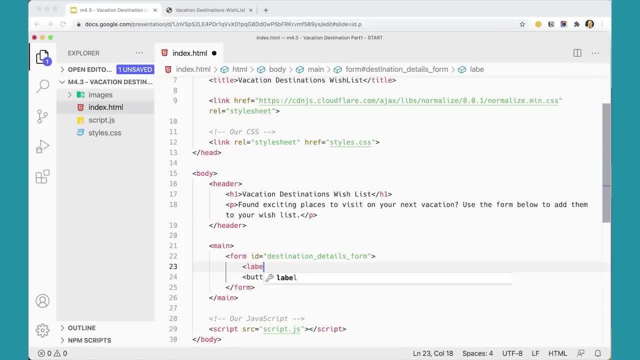 so each of these fields needs a label and a name of the destination, and then we're going to add a label element, destination name, and that takes a for attribute for name and that for attribute connects to the id of the input that goes with it: input type. 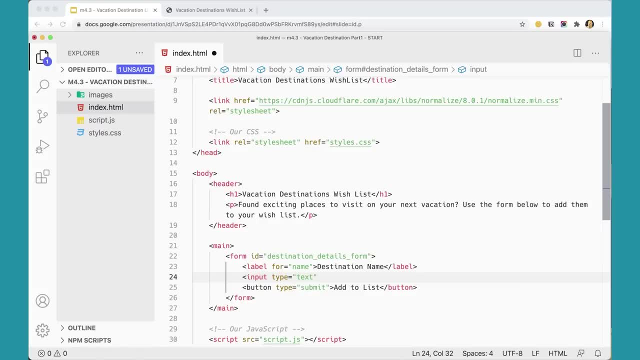 equals text, id equals name. and then also we want to make sure the users use this, so i'm just going to put required: now your browser has to support this for this to actually work. but rather than build in some form validation, which we're going to do in, 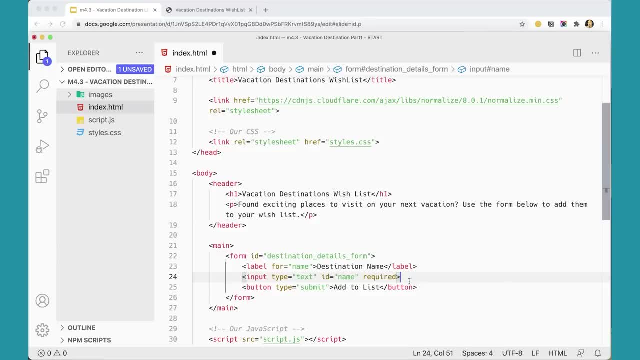 the next course we'll talk more about form validation, but here we'll just use the built-in browser form validation, which isn't perfect, but it it'll help. okay, so now we've got a field here that is required, that has an id that's going to match the for attribute. 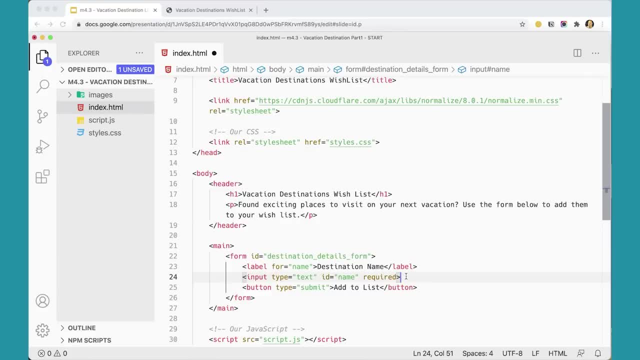 and it's type text, okay, great. and then we're going to need another one label for location- maybe i'll do destination location, something like that- and then, of course, we need the input for that. input type equals text, id equals location and required just like before. there we go. so we've got those two. 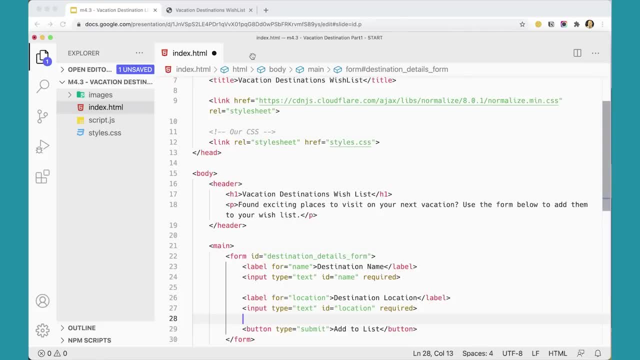 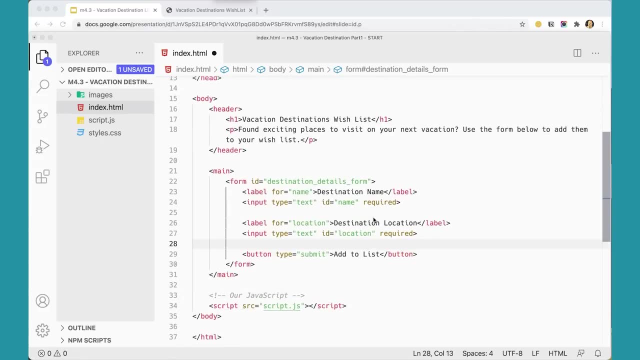 fields in place and from there we can add. we're going to add a couple more fields, i think, yes, we want two more fields, one for the photo, so i'm going to have a label for photo and this one is going to be an input. type equals url, because we're going to paste in a url here. 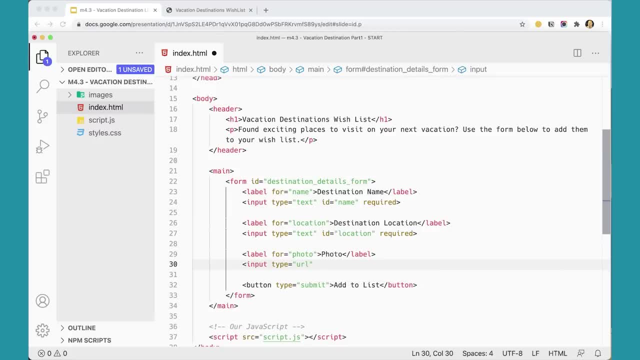 for a photo that's already online rather than upload a photo or anything like that. that would be much more complicated, but we can just very easily find a photo online where we want to put it and put that in there and the id is going to be set to. 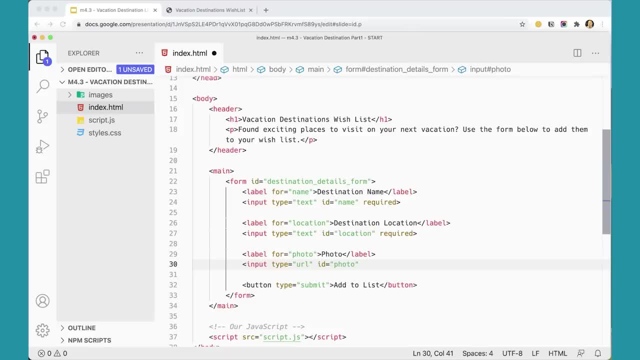 photo, and this one is not going to be required. if we're going to upload a photo, we're not going to be required to upload a photo, and this one is not going to be required, because we can have a default photo in case we need it, and then the last one we need. 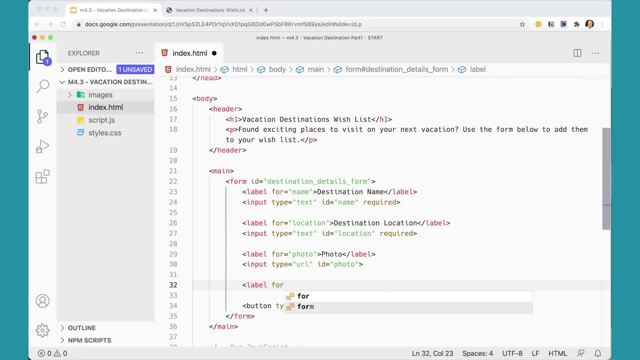 label for description. we'll have a you know, location or destination description. this is going to be a text text area like, so it needs to have an id set to description to match the for attribute. and there we go. our form is basically built. the only thing that would be kind of 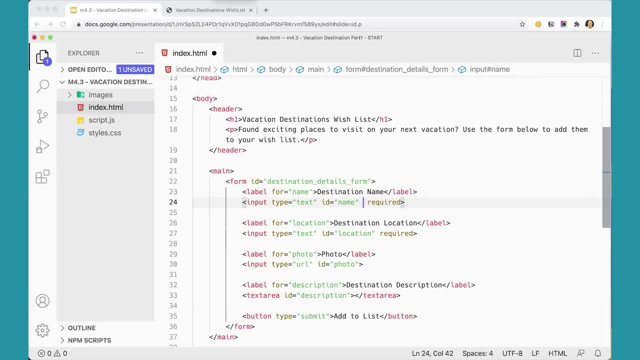 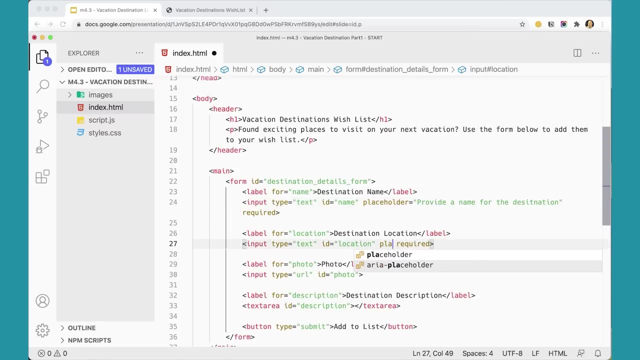 nice is if we had some placeholder text in these fields so we can add a placeholder attribute and set this one to provide a name for the destination. then you will do a placeholder: where is this destination location located for the photo? we can do one there as well. 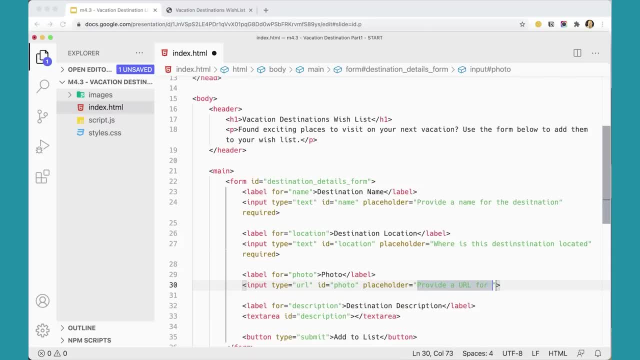 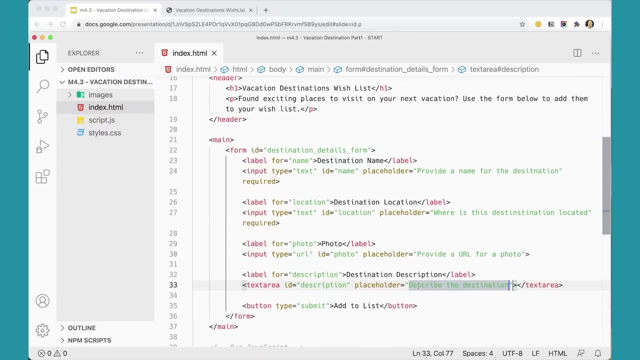 provide a url for a photo and for the description: what is uh, or maybe describe the destination. that gives us a few um, a few things to look for, a few directions for our user, which is use, which is helpful. okay, great, so we've got that, we can save that and we're ready to. 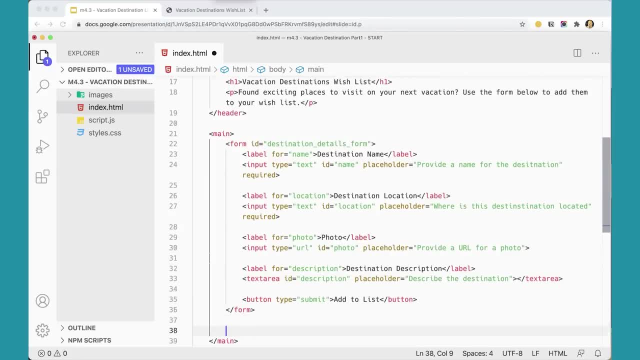 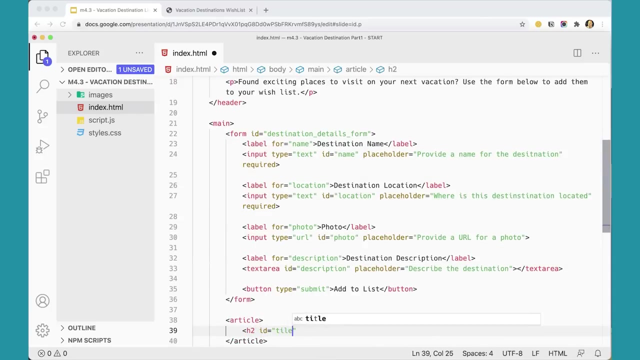 add the element that's going to take the um, the results we put in there. that will be an article, after the format, an article, and then we're going to add an h2 with an id set to title and initially this h2 is going to have a value set to. 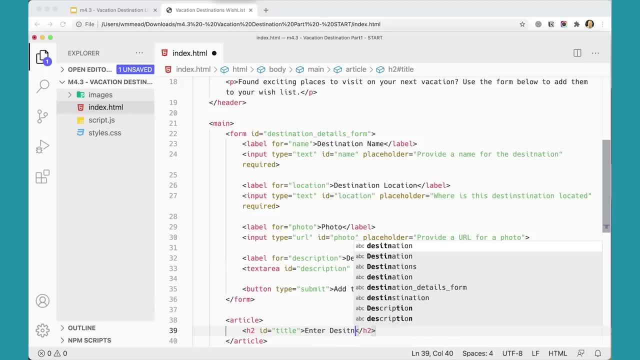 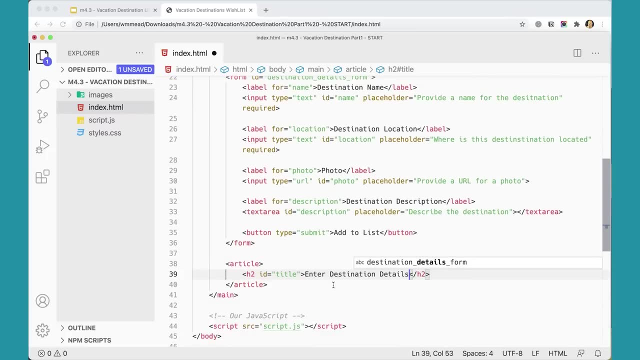 enter test destination details. so that's giving us some instructions there, and then after that we're going to have just a div that's going to be a container for this thing and it's going to get an id just in destinations container, like so, and this div is really going to have in it, you know, the content, content generated. 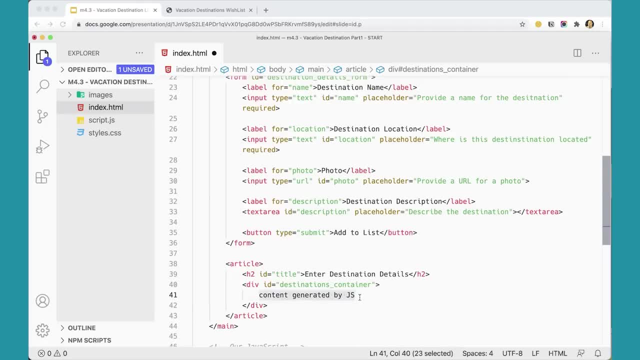 by js. so that's going to get the content that javascript is going to actually generate, is going to go inside this container, and i believe that pretty much finishes the html that we need for now. that'll pretty much finish this off for all the html we need. 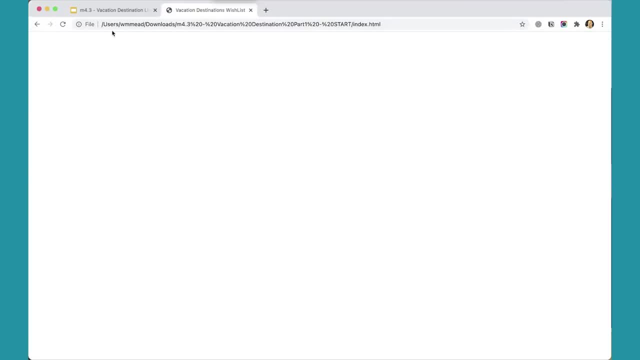 save the file and then let's just go take a quick look at it over here. if i refresh this, you'll see it doesn't look like much. it doesn't look very good. we don't have any styling in here yet, so we'll do the styling next. 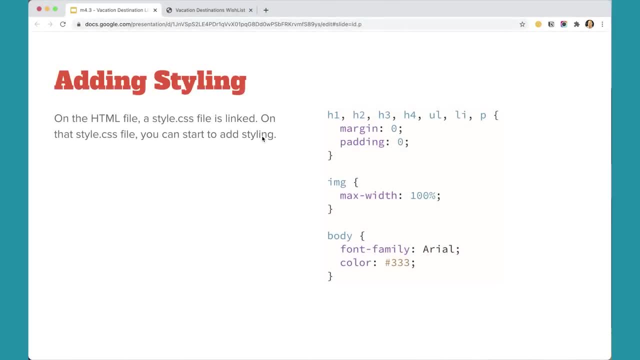 might. we have the html in place and now we're ready to start styling the page and making it look a little bit better. we have the normalized script up at the top of the page, which will help smooth out the differences between different browsers, but beyond that, personally i find it helpful to zero out. 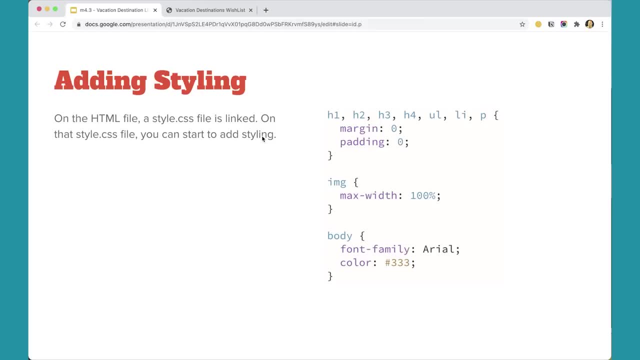 to it to work. so i have here a few reset css things that i think are kind of helpful in general, and this is just my own personal preference. you could leave these out if you wanted to, but generally i think they help with sort of zeroing out some of the base styles that 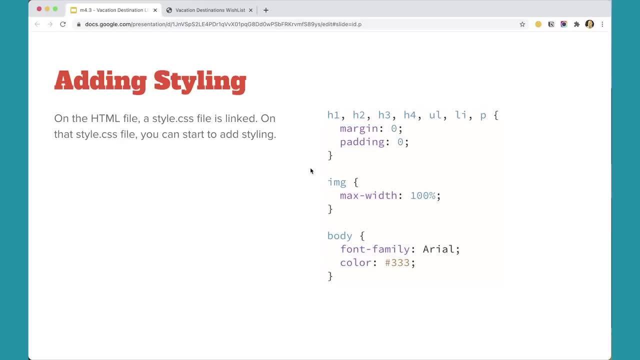 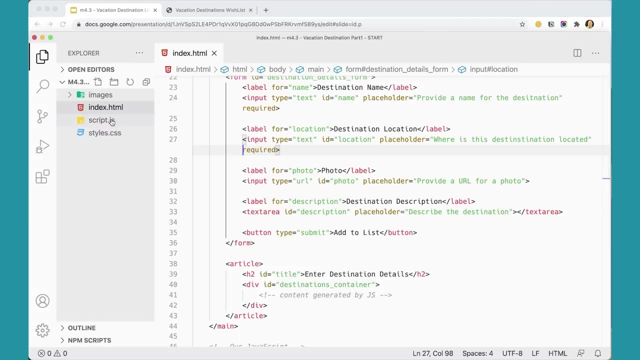 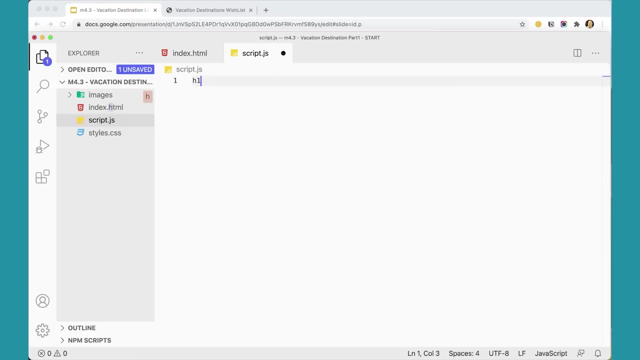 cut that most browsers display by default, so i'm going to go ahead and add these in and over here. i'm going to add on my style sheet here a rule for h1, h2, h3, h4, ul, li and paragraphs. i don't know what's going on with that. there we go. i'm putting this on the script page. 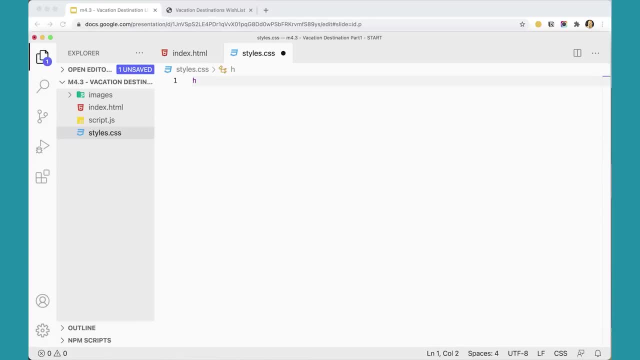 styles: h1, h2, h3, h4, ul, li in paragraphs: margin padding zero, padding zero. that just kind of gets rid of the margin and padding of those elements. it's also helpful to say img max width: 100 um. i think that's kind of helpful to make sure images don't. 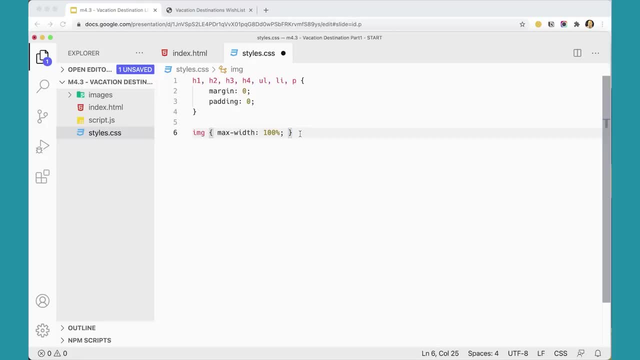 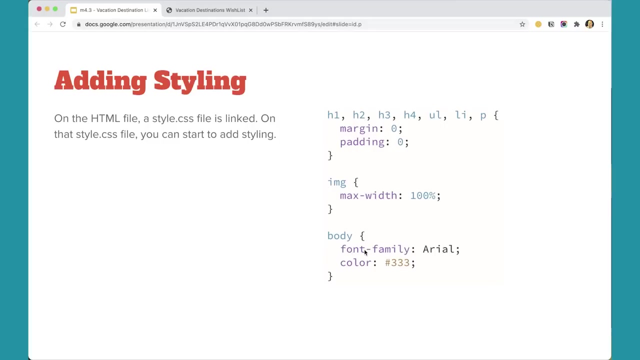 bust out of their containers. if you have a, if you put an image in for a url that's that's too big to fit in the container, it'll overflow it. we don't want that to happen, so we'll set that as well. and then i also have over here just some styles for the body i'm going. 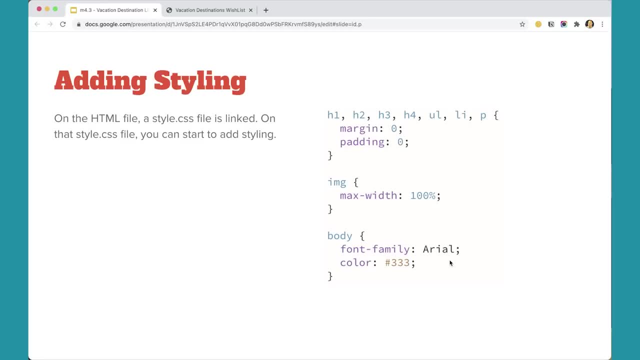 to set the font to ariel. ariel is the font that most computers have, so it'll work pretty well, and i'm going to set the color to a dark gray, the color of text to a dark gray in this basic rule here. so let's just add that really quickly as well. so i'm going to have body. 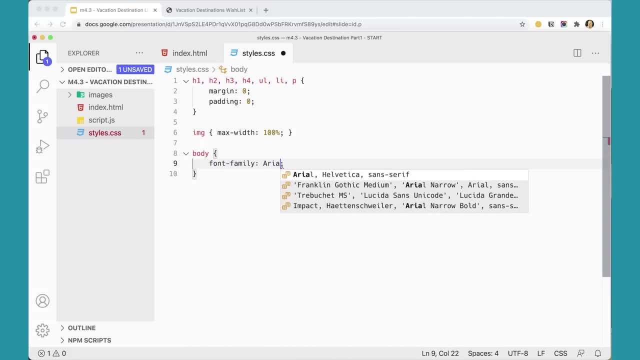 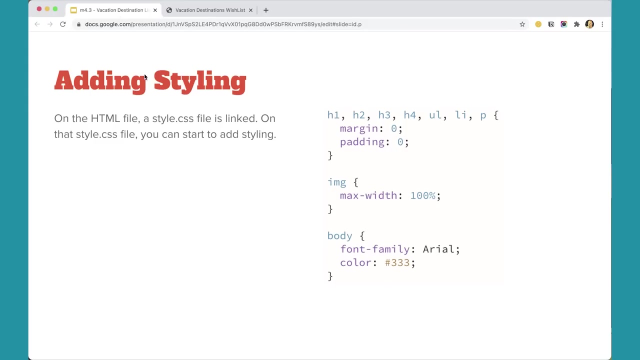 font dash family ariel, and color pound 333. and already you'll see that the page is starting to come together a little bit with some of that styling. there we go notice that we've lost a bunch of the margin and padding on those things. okay, great. 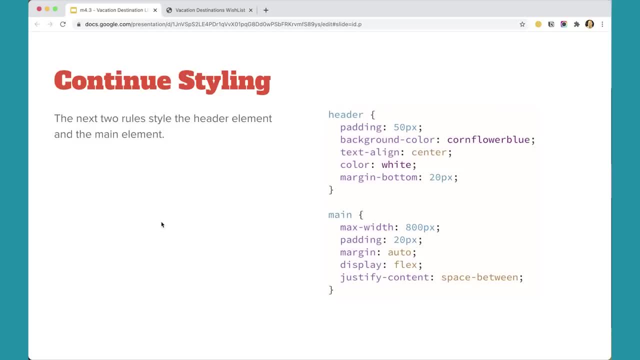 next we're going to style up the header and the main content to kind of get them to look the way we want them to look. so, header, i'm going to set the padding background color, text align, center, the color of the text in there and then the margin on the bottom. so let's do it, go ahead and do that. 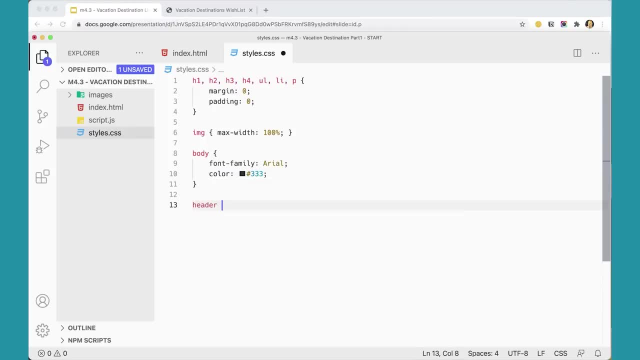 and we're going to add the text and then we're going to add the text header padding: 50 px. background color: using this cornflower blue. we're setting the color of the text to white text align center. i put a margin on the bottom margin: bottom: 20 px. 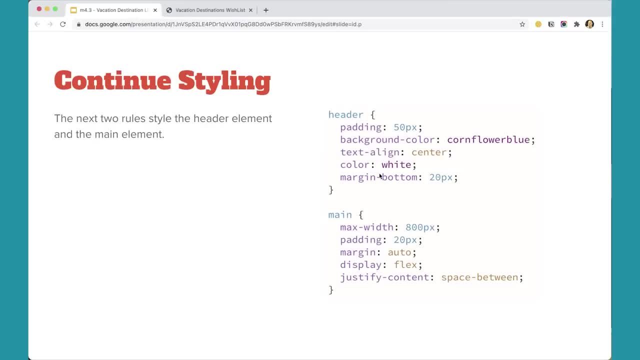 and anything else that i did over here. yeah, that's all good, all right, good. and then for main, we're going to have a max width: of 800 pixels padding, 20 pixels margin, auto that will center it on the page. display flex that will make the two items in there sit next to each other and justify. 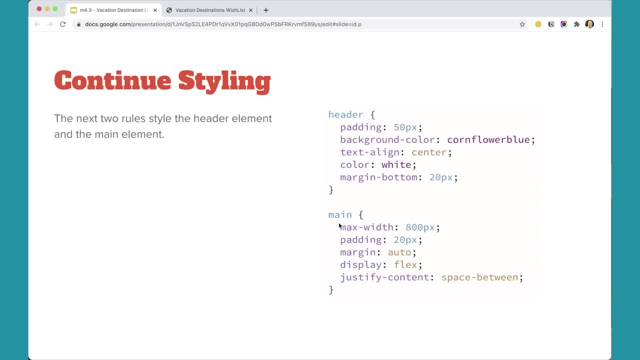 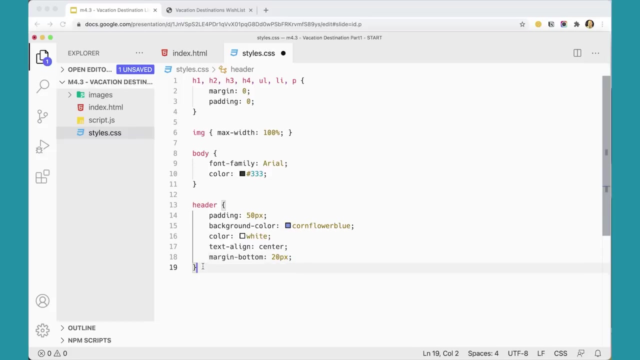 content space between, and then we'll set sort of percentage width or specific width for those two items that are going to sit next to each other on the page there. so let's go ahead and add that in main. max width: 800 px. it's kind of a narrow page, but that's okay for what we're doing. um display. 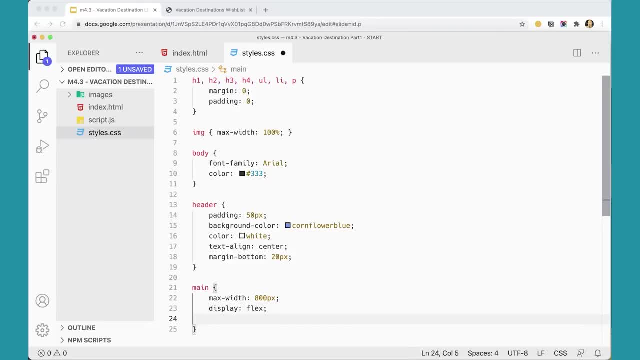 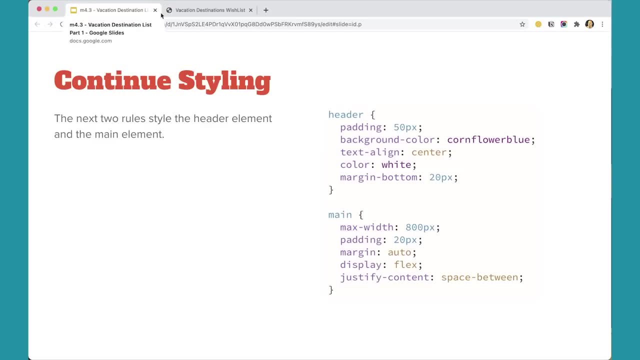 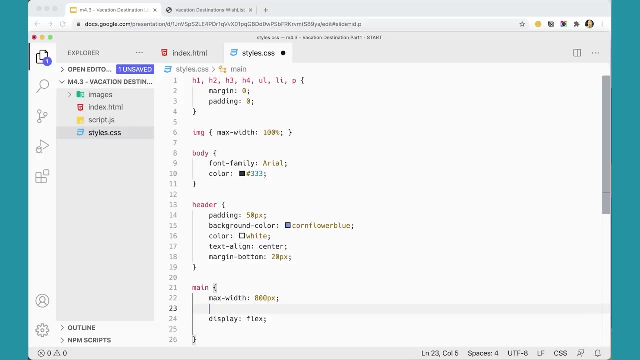 flex that turns it into a flex box. and i did some stuff with margin and padding. that i do here. padding 20 pixels margin auto. put that above. actually it doesn't really matter, but padding 20 px margin auto. there we go, and then with display flex, we'll do justify content. space between: 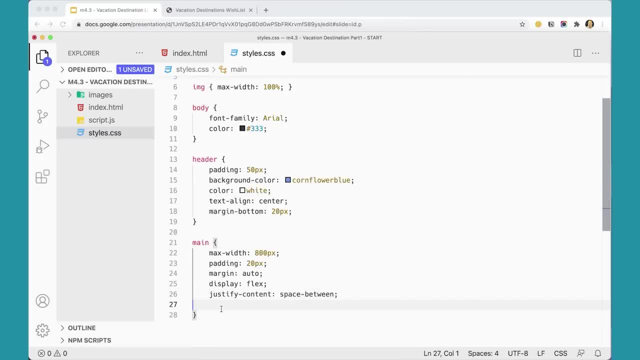 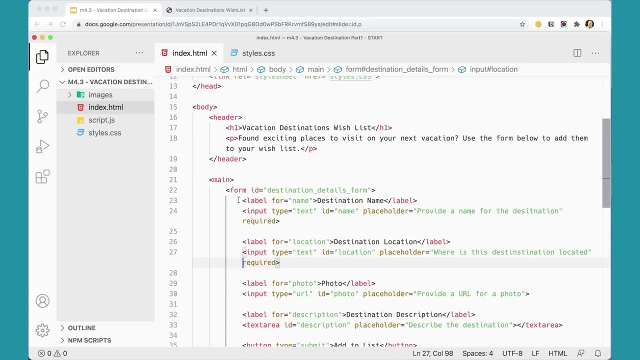 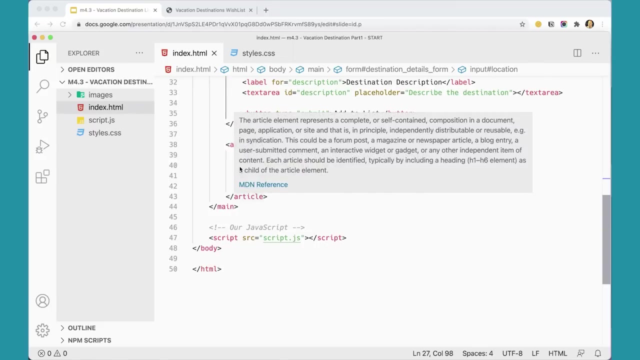 the two items which we'll put a gap between. those two items, the. the two items that are going to go next to each other are the form on the left and then this article on the right. those become flex items. they're going to go next to each other to sit. 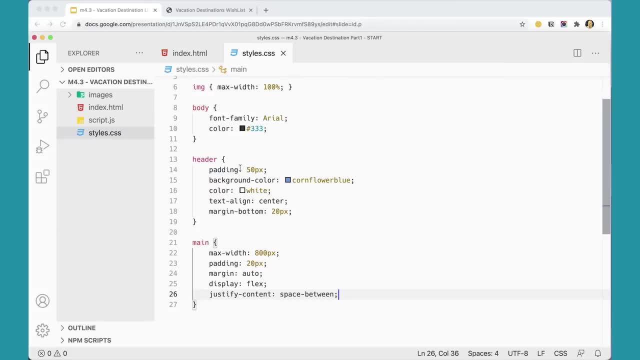 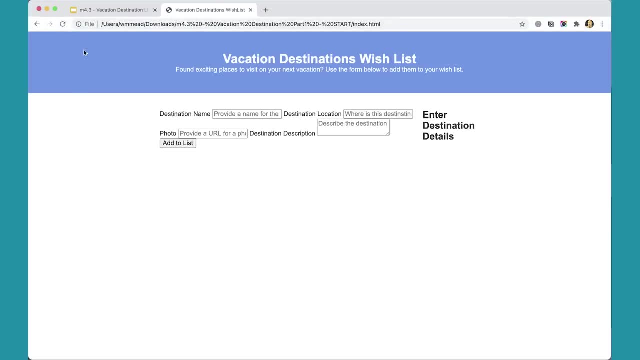 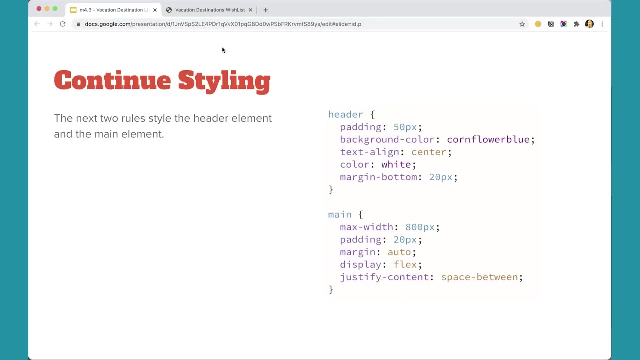 to sit next to each other in our design. so, um, just like that, even with just those two rules, you'll see it's starting to, uh, to come together a little bit. more bit there, not very much yet, but it's starting to come together. okay, great, we'll pick up the styling in the next video. 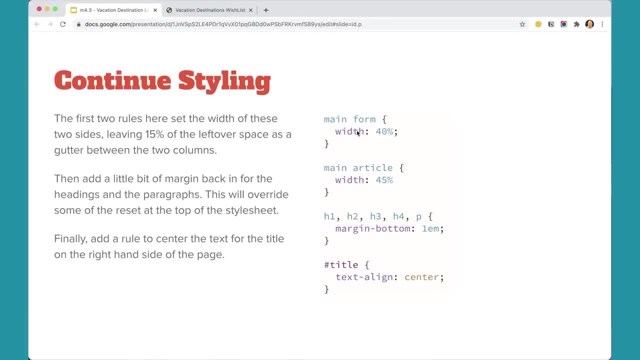 okay. so next we're going to set the width of the form and the article respectively. we'll add some margin back in the bottom of these elements, uh, so that they have so they start to look a little bit better. and then the title is going to get text aligned to the center. 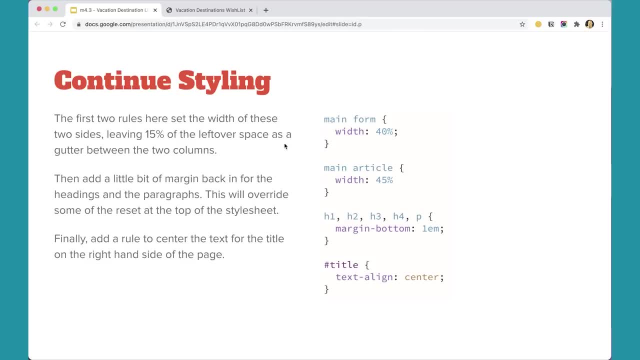 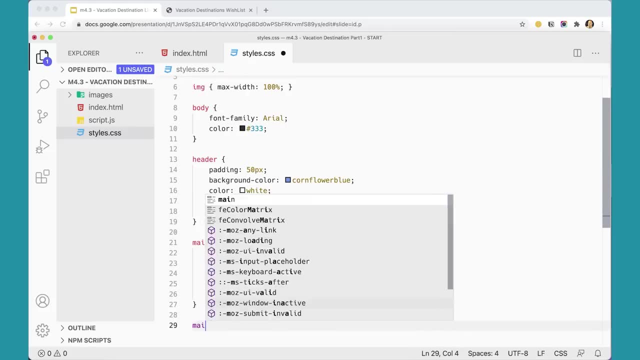 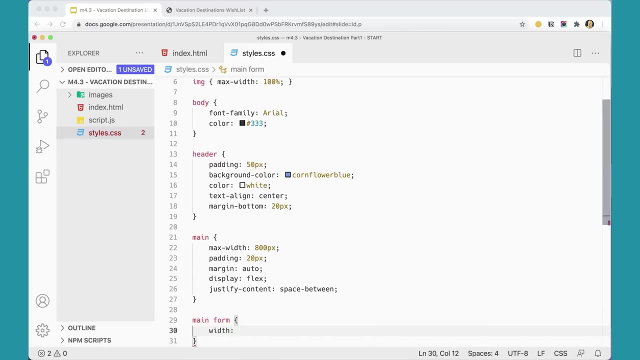 so we'll be able to do all of that here. so let's go ahead and add that into our style sheet. here, mainform, we'll target the form itself with 40 percent, setting it up a little bit to be responsive, but not entirely. main article is going to be with: 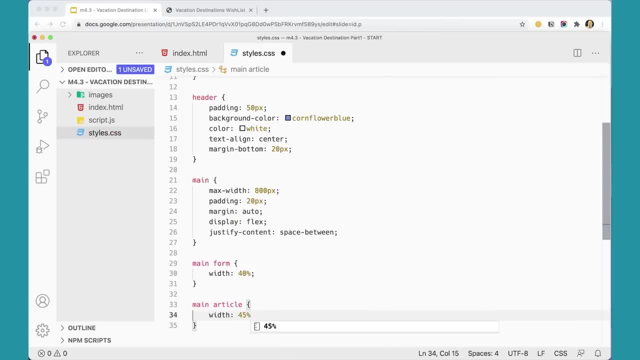 45, so that adds up to 85, which means that 15 will be left to be the gap between those two, to create a little bit of a of a gutter between these two columns here. so we got that in and then we can just put the margin in the bottom of these elements. 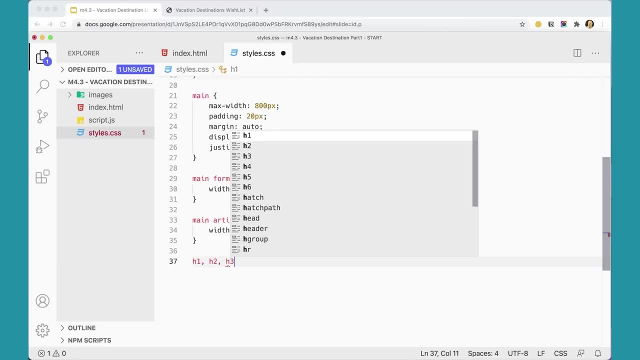 h1 comma, h2 comma, h3 comma, h4. we have all those. we might margin dash bottom 1m, you might be wondering. well, it seems kind of silly to take the margin out up above and then put it back in down below, but i found that i get a lot more. 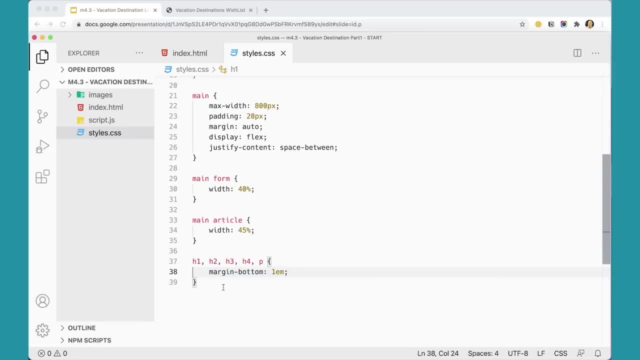 control over the look of my look of my pages and the visual spacing between things. if these elements only have margin on the bottom and not margin on top and bottom, which is what they get by default in most browsers, okay, so if we save that and check it over here, you can see it's starting to. 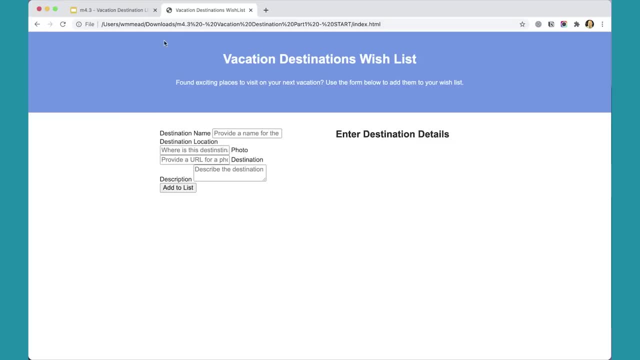 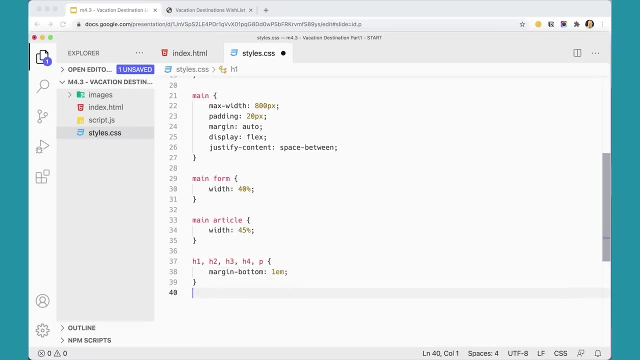 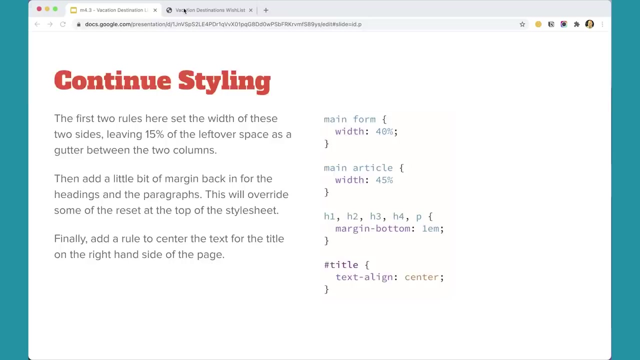 come together a little bit more. but the last thing i was going to do is i'm going to go ahead and do is center that title over there. so we've got um pound title text align center. there we go. let's see what else we need to do for styling. 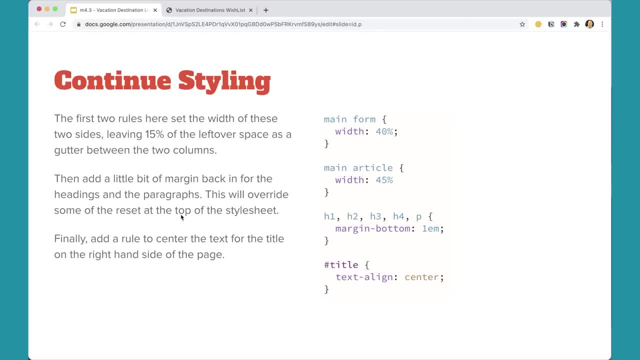 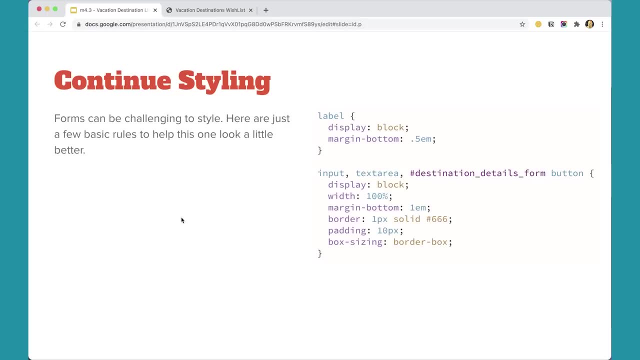 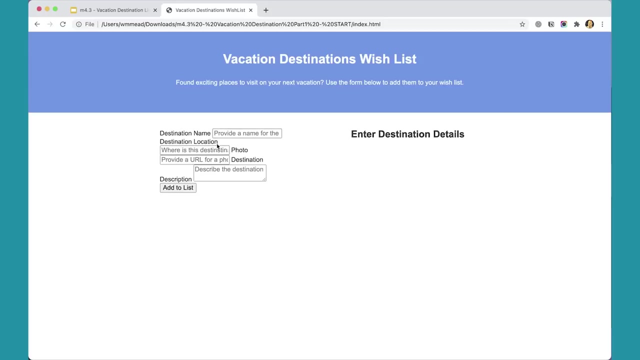 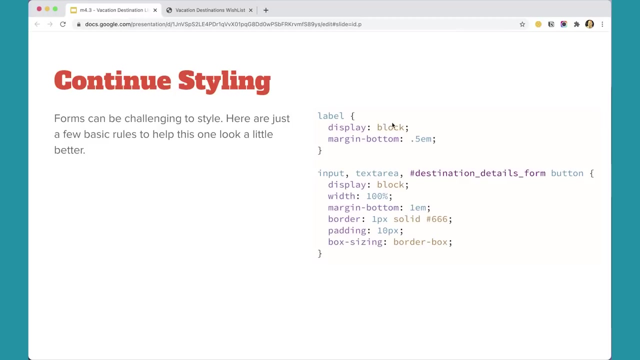 got that going, so that's centered over there now. that's great, and then now we can um slide some more forward down. here. we've got a map, see essentially a66 plus. i really liked this one today and i'm so excited to speak about you today. um, we're just gonna do a. little bit with forms. um, and with forms, you can spend a lot of time designing forms and styling them. we're just going to do a little bit right now. what you should notice to begin with is that, by default, form elements are in line, or phrasing elements will go next to each other, and we don't really like that. um, we wanted to kind of stack. so if you set them the display block and 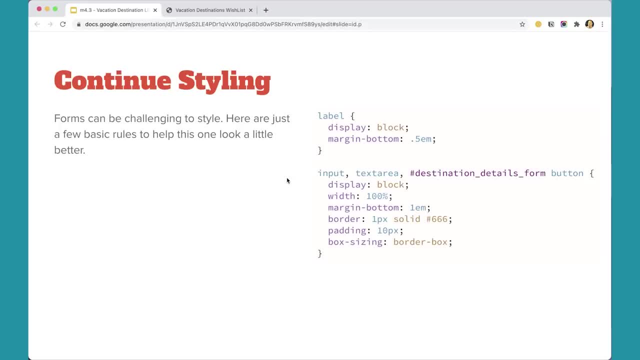 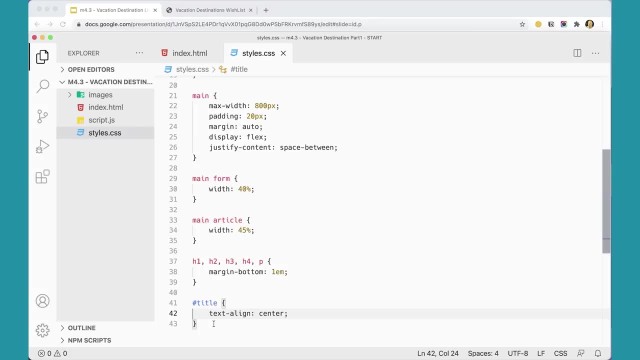 then work with them a little bit easier. you just draw desgin and then it easier to work with, okay, so, um, let's go ahead and add these rules in here for the label. we're going to tell that to display, block and put a little bit of margin on the bottom margin bottom. 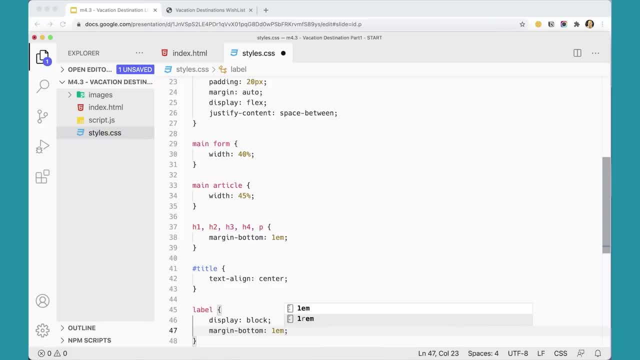 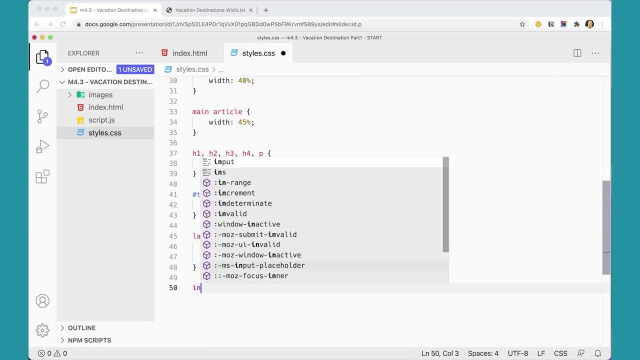 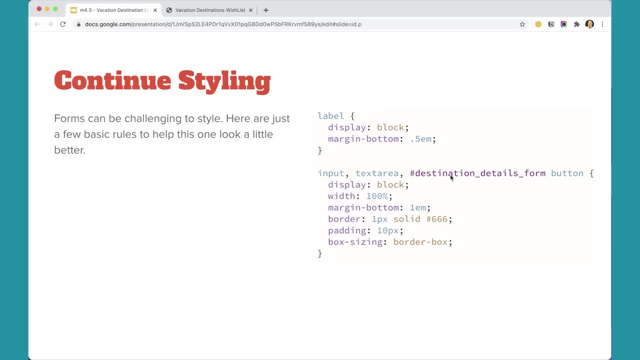 um, when m is fine, that's cool, so that'll work. and then for the other thing, we've got input, we've got the text area and we've got this um form. what did i have over here? i called it, um, oh, just the destination details form button. so this is just the button inside the form. 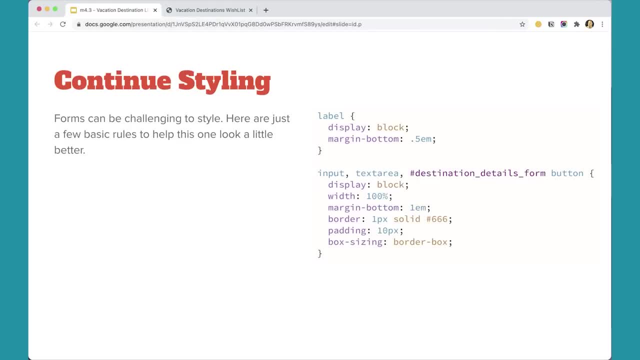 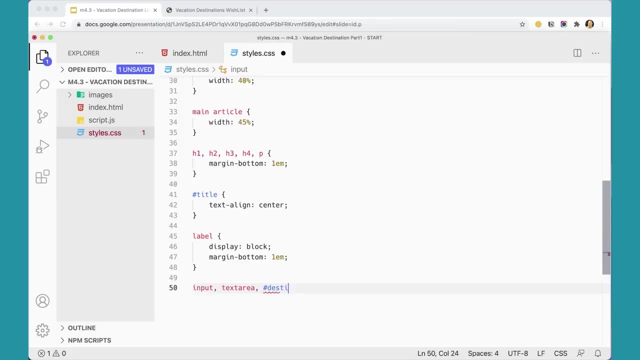 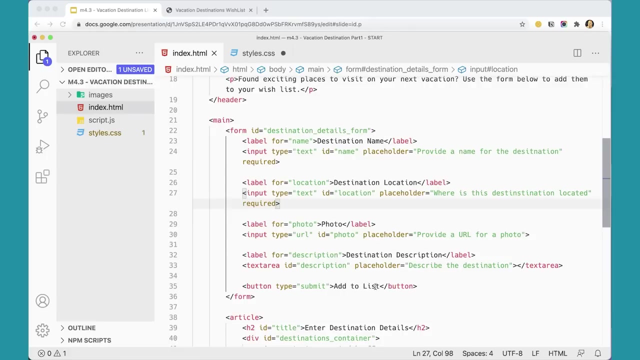 and i'm being specific because we might end up with another button later and destination details form button. so that button, that specific button that's in over here, so that's this form, destination details form, and then this button down here. so i didn't put an id on it, so 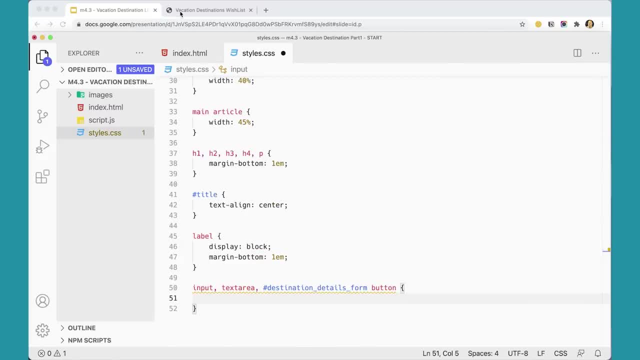 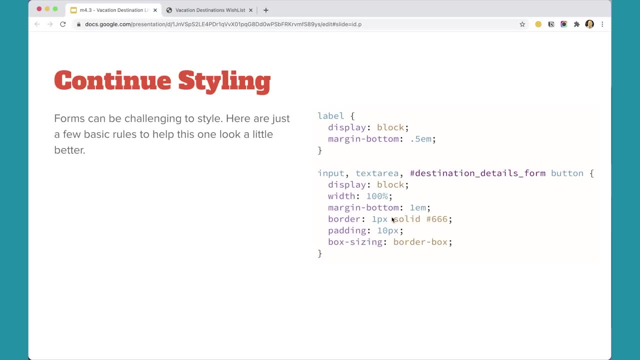 being kind of specific there and what we want to set is just um display block with 100 margin, bottom 1m. i put a little bit of border on it with a sort of medium gray um and some padding and box sizing border box. so let's do that. 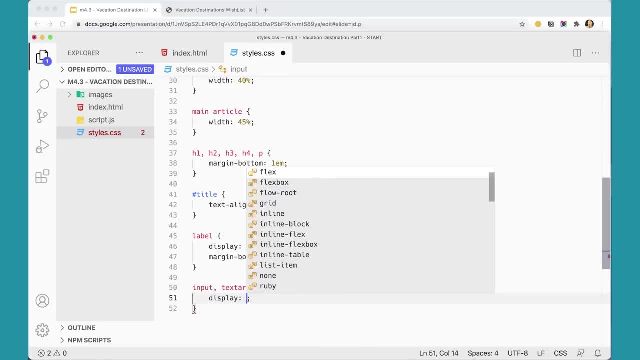 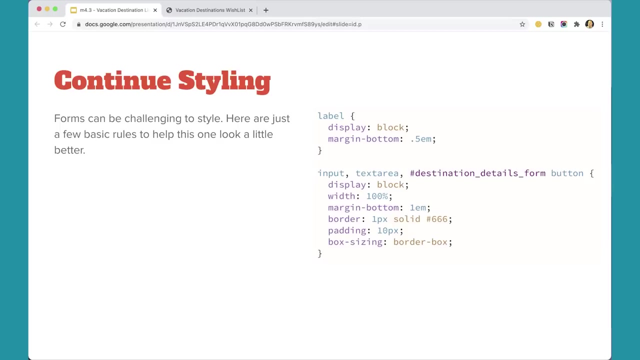 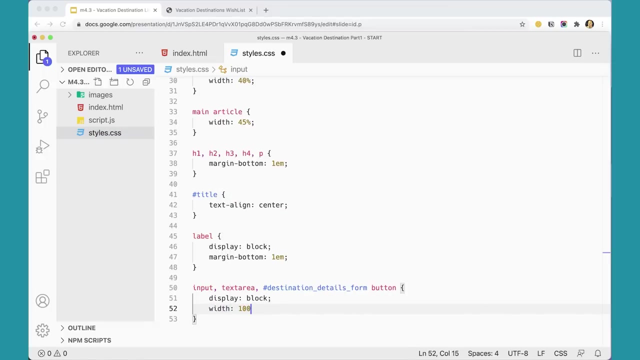 display block that will make each one take its own line. um to do to do. what was it again now like wrong one? um width 100. margin bottom 1m. margin dash bottom 1m. you've got that border 1px solid and 60. 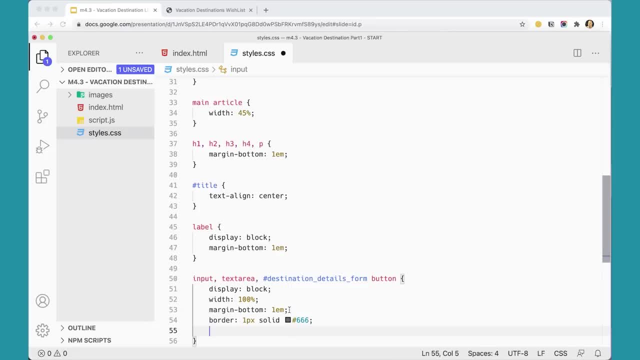 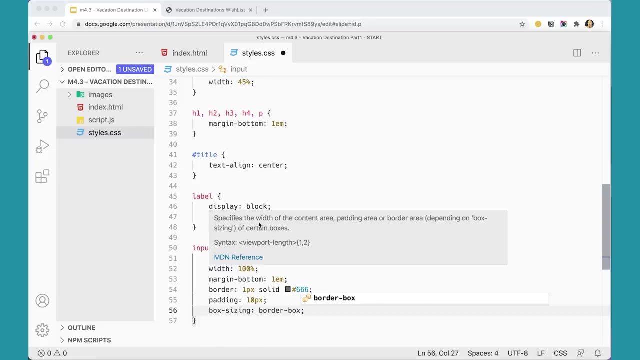 6: padding: 10 px box sizing border box. what box sizing border box does is it makes the padding and the border part of the width of the element. remember, we set the width to 45 percent, so we don't want to extend beyond that size there. all right, cool, let's take a. 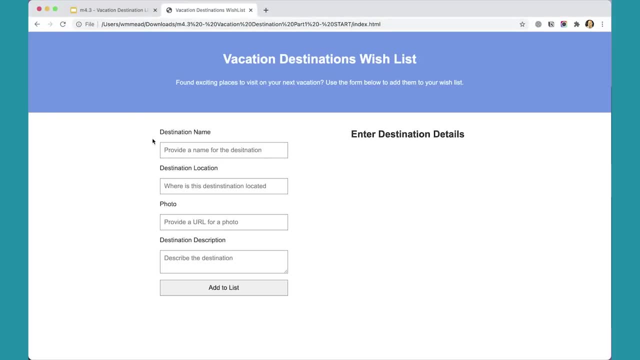 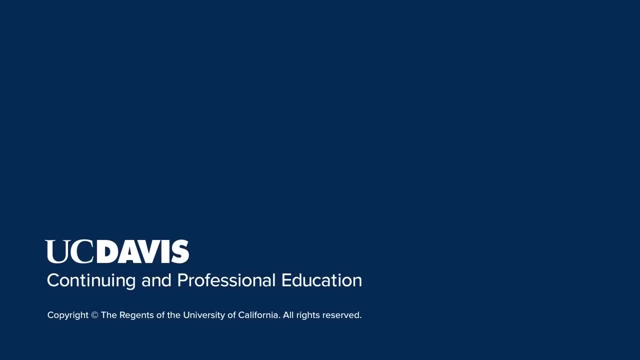 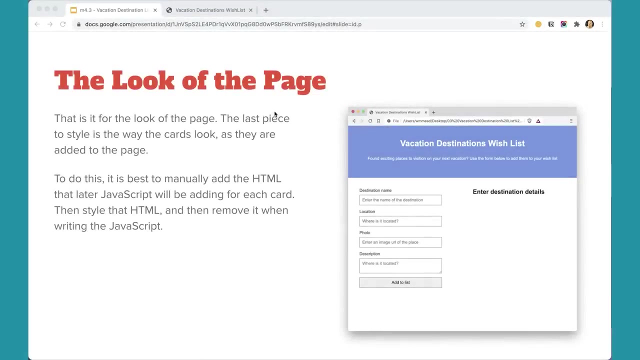 look and see what that looks like over here. well, that's looking much better, much cleaner. we will finish up the html in the next video, i mean the styling. in the next video. we're going to add cards dynamically using javascript, but we want to know what they're going to look like, so the best way to do this is: 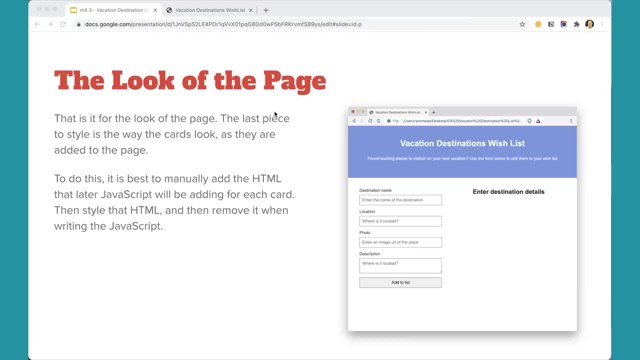 to add one manually. add a card that would get added by javascript with all the correct html style, that so we know what it's supposed to look like- and then remove that card. so that's what we'll do next. so we're going to start by going back and adding: 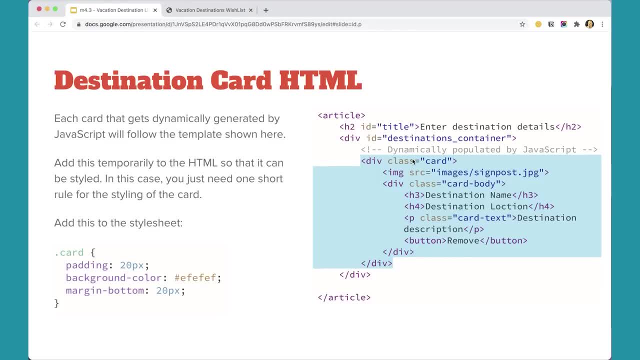 just a little bit more html. so we need a div with a class of card and an image with the sign post, and then in there we're going to have the card body with an h3 and an h4 and a paragraph and button. so we do have another button here, okay, so let's go in and add this into our. 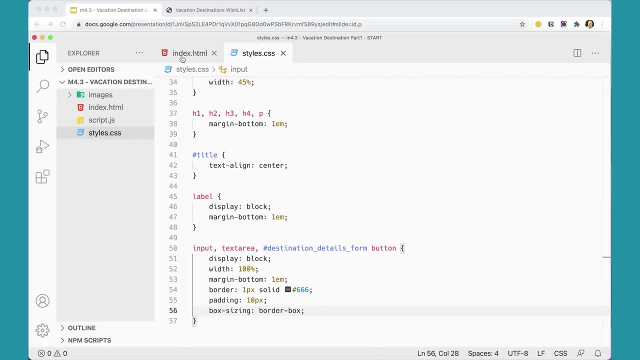 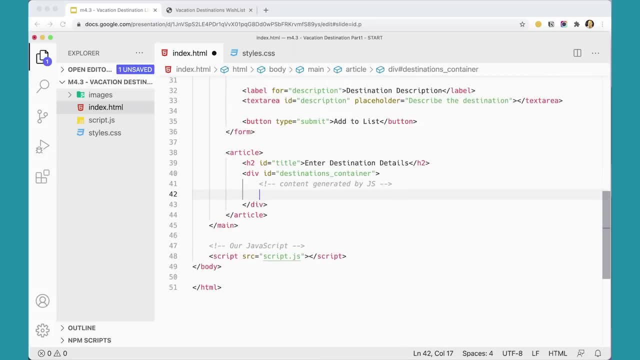 html over here. it's going to go down here inside this generated content by, by javascript. here we're going to hit: do div class equals card. this has to be a class because we're going to have multiple cards, right, we're going to have multiple cards on the page, so you can only use an id once. that has to. 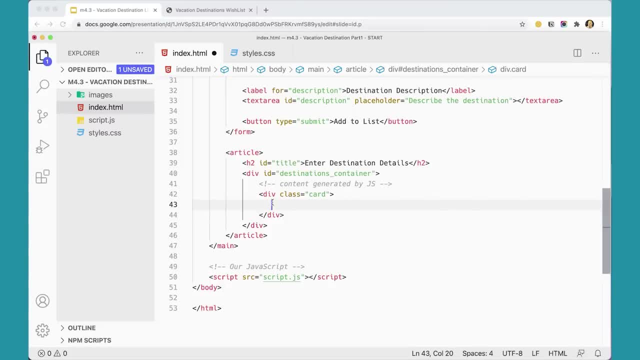 be a class, then let's add an image images sign post. i'm not going to put an alt tag on it at the moment, so we've got that image and then and then we've got sort of the card body coming next. div class card dash body. 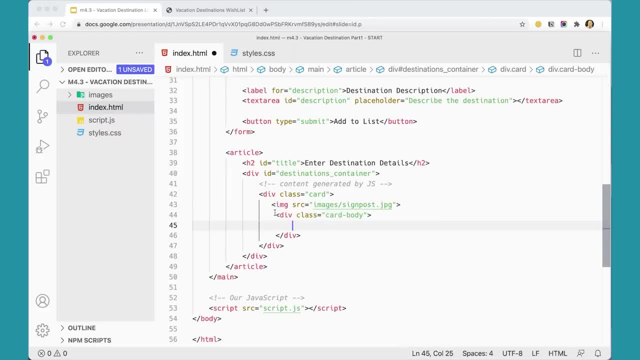 i don't know why that is slightly misaligned. that's right. maybe it's this one that's. inside there we go div class card body and then inside the card body we're going to add h3, destination name, and then i'm going to do an h4. 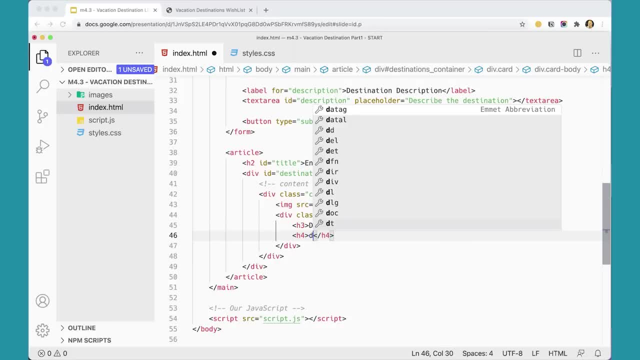 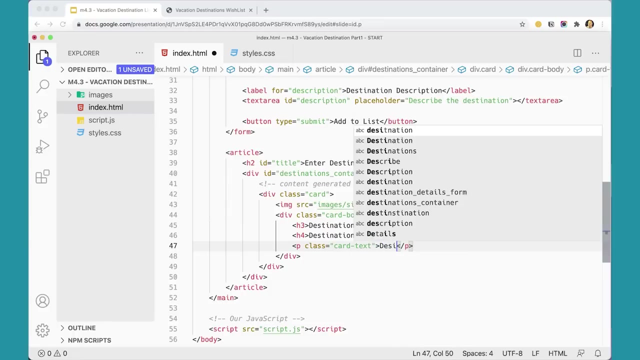 destination location- and then we're to add a paragraph p with a class set to card text- destination description- and then we're going to add a button that will allow you to remove the card. if you need to. we'll have a feature that will allow you to take a card off. 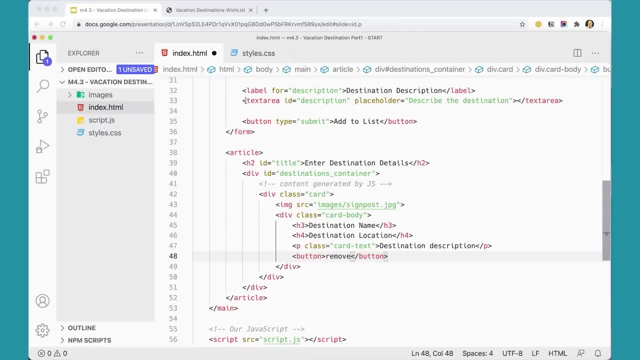 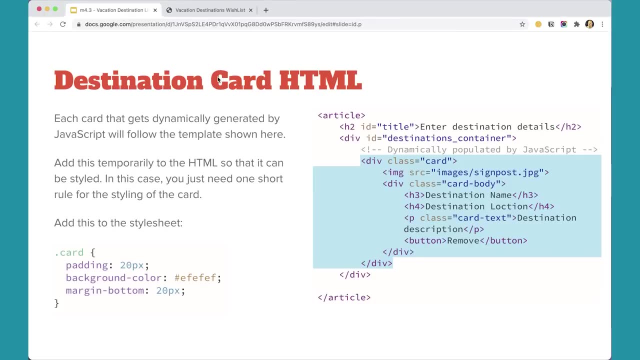 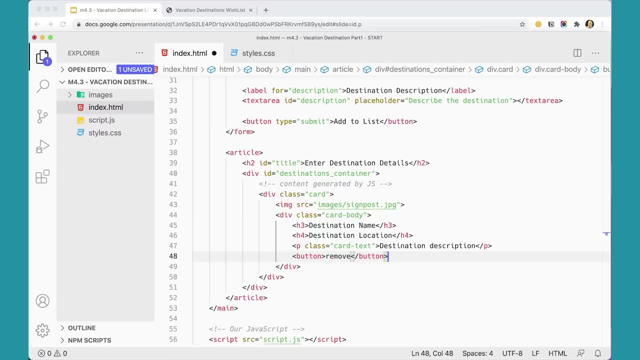 so we'll add that button there and i believe that's what we need for the html. let's take a look over here, possible? so we've got all of all of the HTML for that card in. it won't look particularly good. let's see what it looks like. 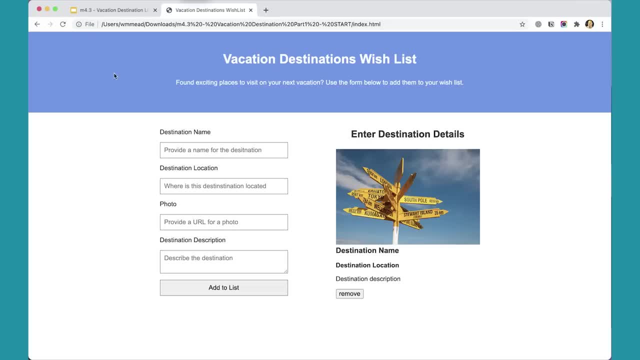 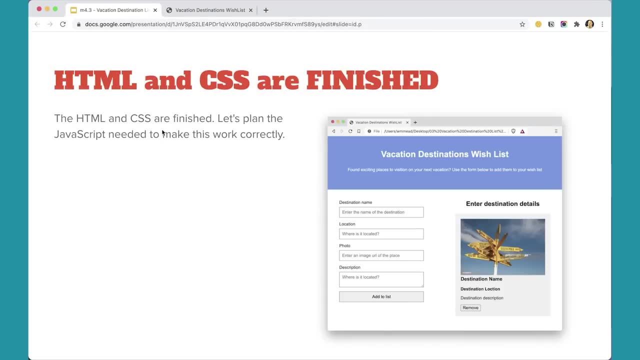 doesn't look terrible, but it looks okay, but we might want to do a little bit more with it. actually, it's fine for now. we'll leave it the way it is. we've got kind of our basic card in there, although I do have a background color in there. 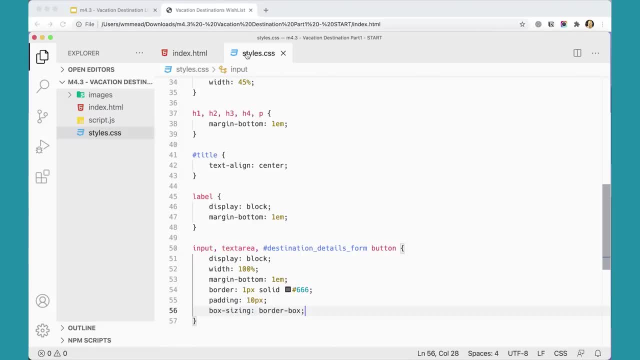 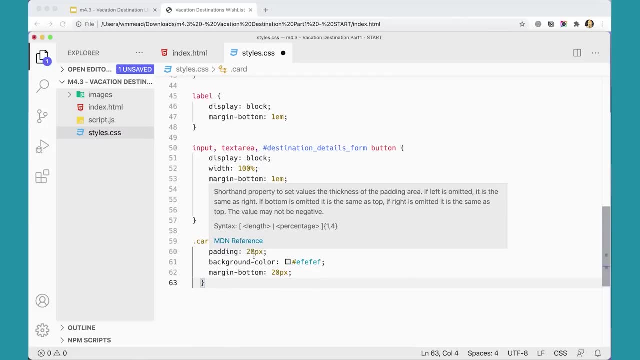 don't I? let's add that. let's add one last rule down here for the card. I'm going to just give it a little bit of padding, set a background color and set up some margin on the bottom, and that should look good. let's take a look at. 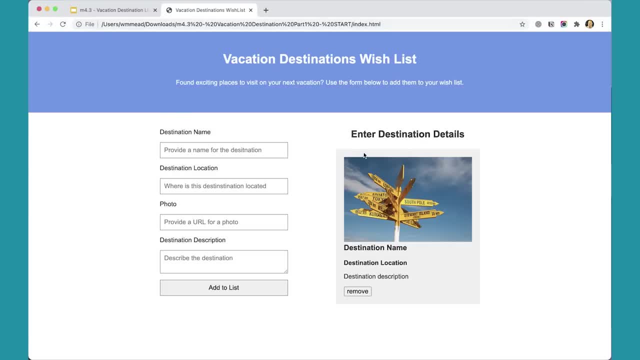 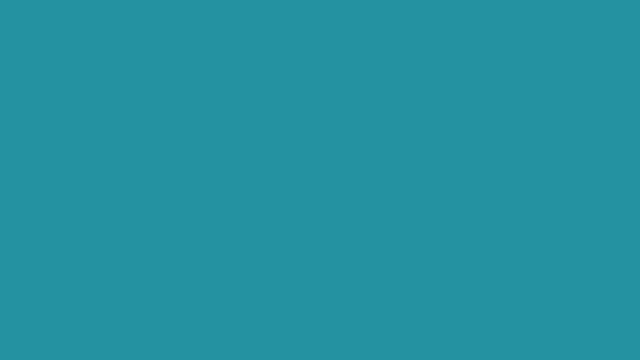 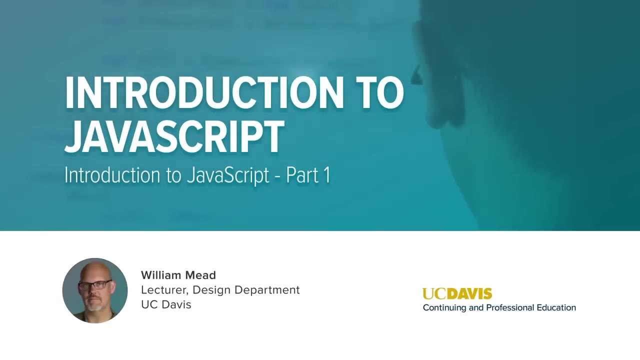 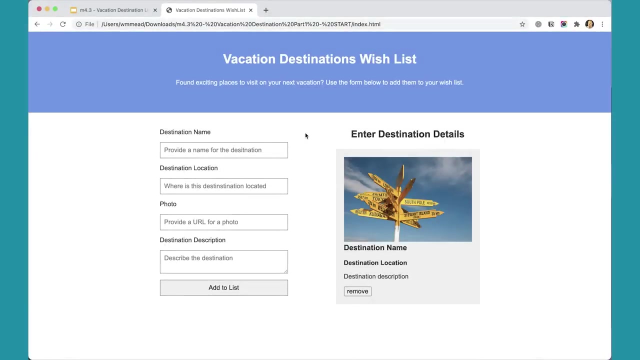 see how that goes, there we go, so now we've got a card that's looking good. ultimately, these are going to be put in through JavaScript. the HTML and CSS is in place now, and we have. now that we've got that in place, we can start thinking about how this little application is going to work. essentially. 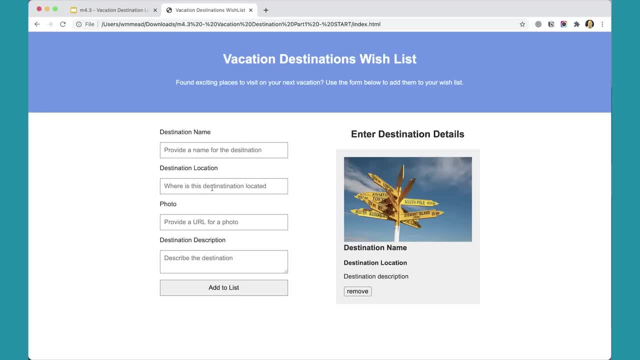 users going to type in a name and a location and provide a URL for photo in a little bit of a description here, and then that will get added. that cart will get added to the list over here. let's take a look at a little bit of a flowchart to sort of see. 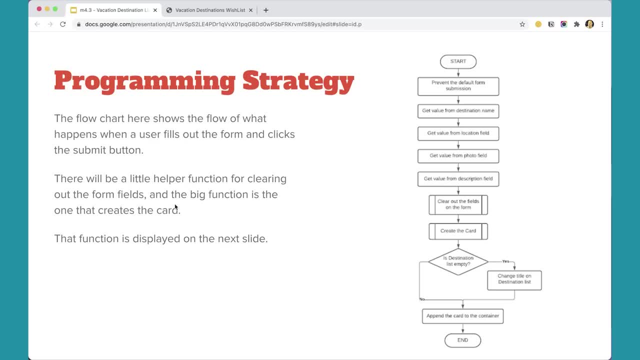 how this is going to work and how we're going to kind of make that all work out here. so over here the right side of this page, you see a. We have a little program here that, when it starts, we're going to, when somebody fills out that form, we're going to prevent the default form submission. 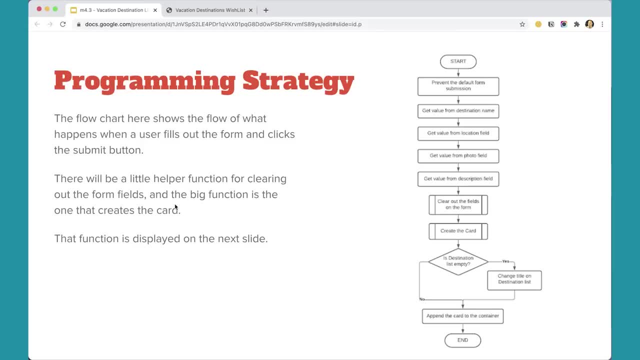 We're going to get the value from that destination name, the location field, the photo field, the description field, And then we're going to clear out the fields in the form, create a card, create that HTML and check to see is the destination is empty. 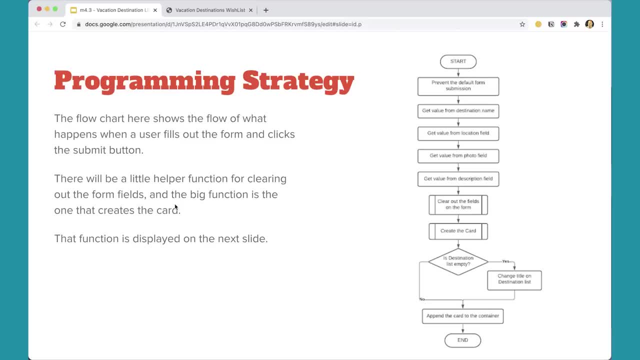 Is the destination list empty? If it is, then we're going to change the title on the destination list up at the top. If it isn't, then we'll just append the card to the container. In either case, we'll append the card to the container and we'll be able to move on from there. 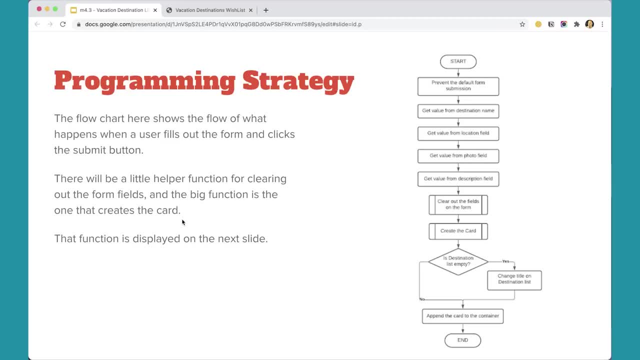 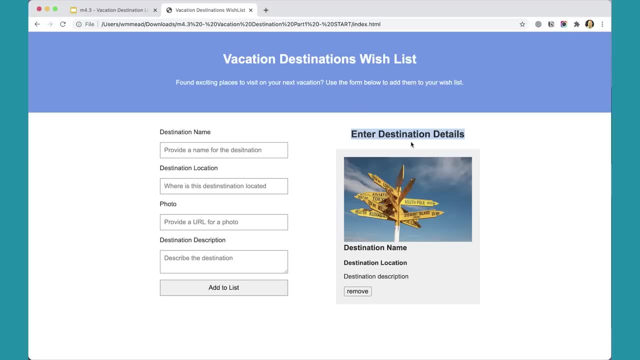 Okay, so that's going to be the basic strategy for how we add stuff to the page. So the first time we add something to the page, this title is going to get changed, but otherwise it's not. So that's the only. 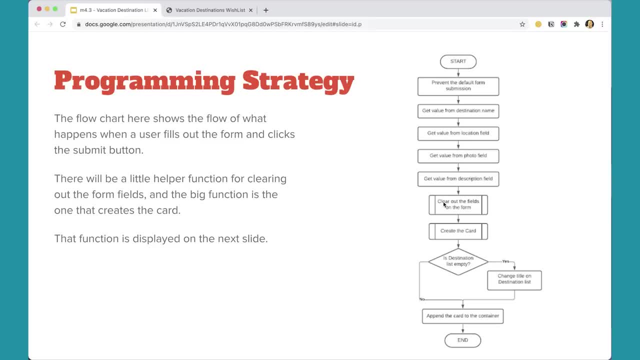 That's the only thing that's kind of going on there. that's interesting. These are going to be the little helper functions: Clear out the fields and then we're going to have a helper function that's going to create the actual card. So those are the next functions we need to look at here. 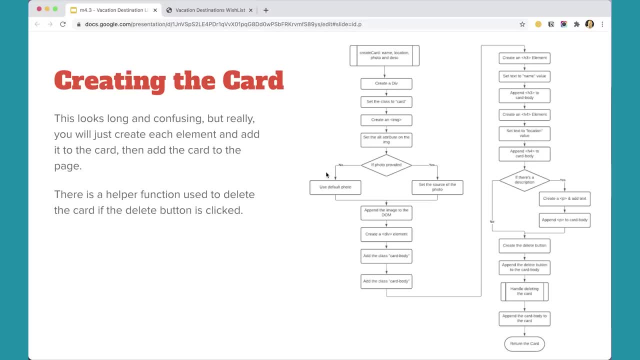 The creating the card looks like a really long function, but it's very sequential And basically we're just going to create a div and set the class to card, create an image tag, set the alt attribute on the image tag And then, if the photo is provided, we're going to set that source to whatever the URL is. 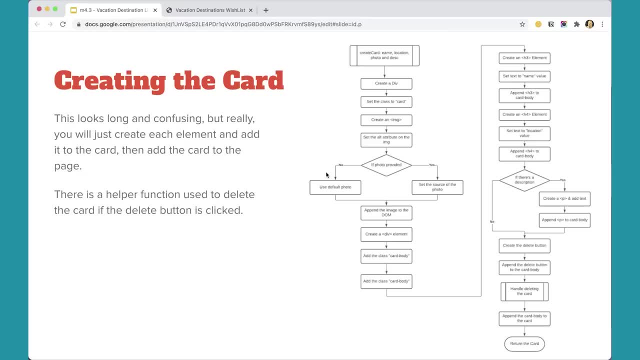 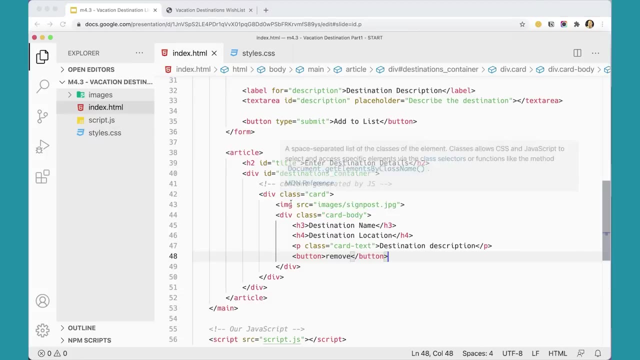 If it isn't, we'll use the default photo and then assign that to the image element on the DOM that we just created, And then we'll create a div element. So basically, we're creating the elements manually or having JavaScript create them to create these elements here. 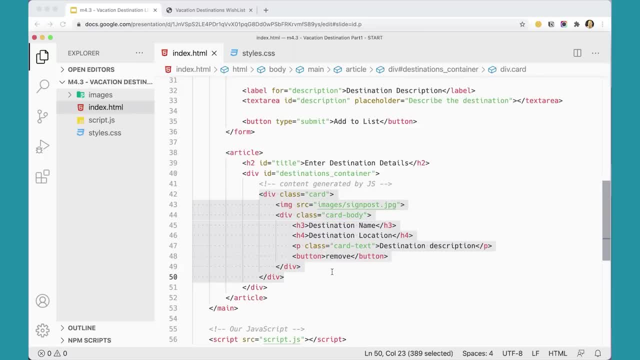 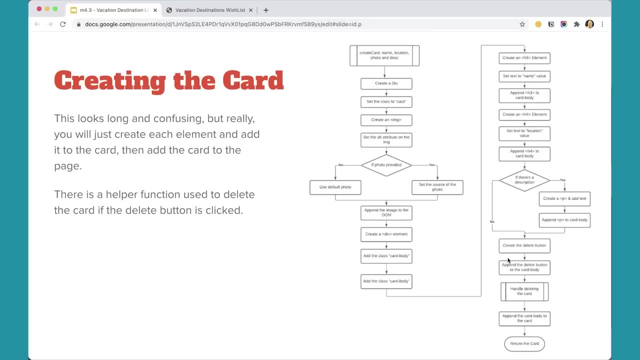 We're creating all of this HTML here for each card. We're going to create that, We're going to create that information and then we're going to stick it on the card And that's what's going on here. And you'll notice, down here we've got another helper function here for deleting the card. 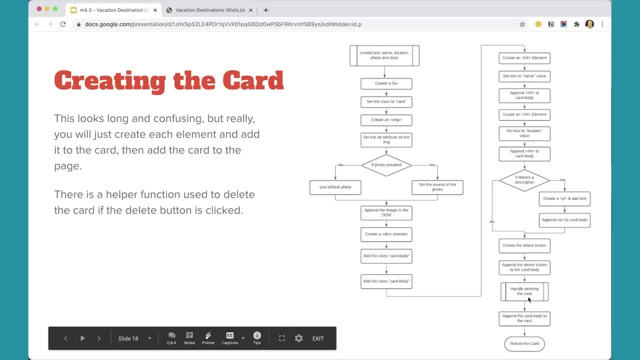 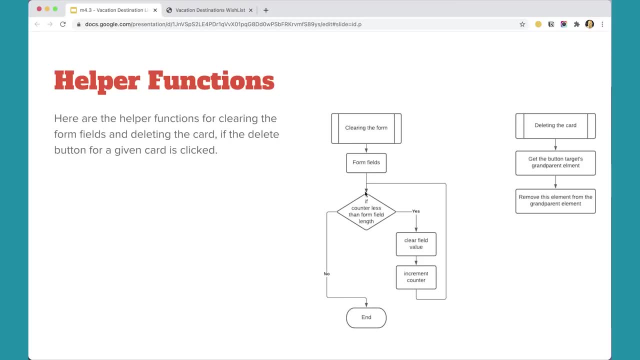 So if somebody clicks that remove button, then we need to be able to handle that as well. So let's take a look at that really quickly. So we've got a function here for going through the form fields and emptying out the form fields. 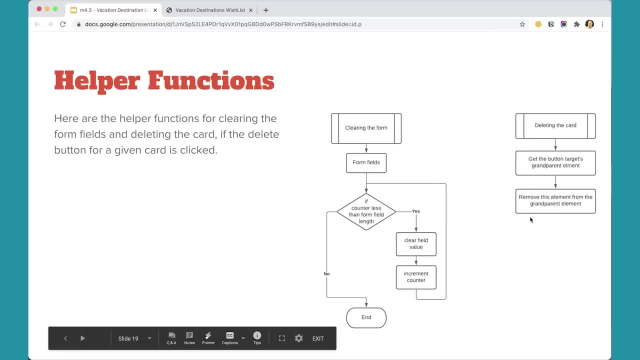 And then we've got a little function here: We're deleting the card if we want to delete the card. So we've got a number of pieces here to write in our JavaScript to create this little application, this little functionality for this destination list. 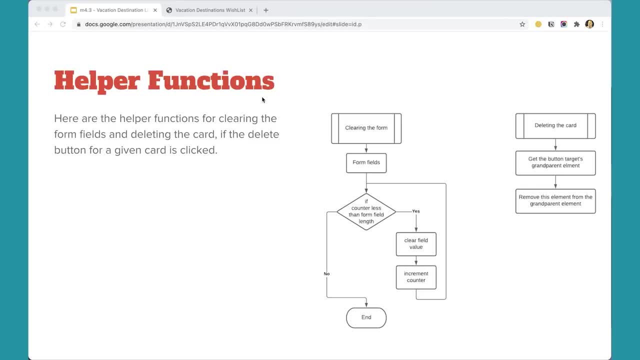 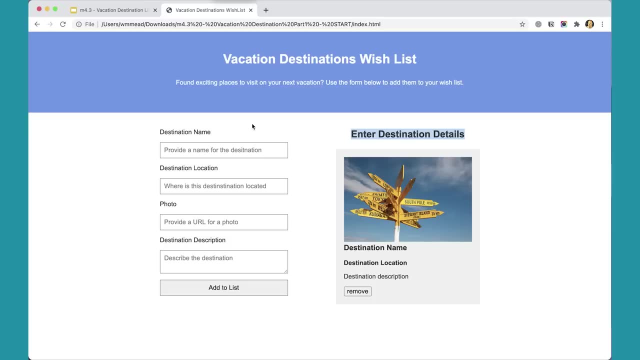 And that's it for part one. We've created the interface that we're going to be using, And you may be wondering why we spent all this time in HTML and CSS, but it's really important to understand how the HTML and the CSS interact with the JavaScript, because all three come together to make the full interface and to make all the functionality work. 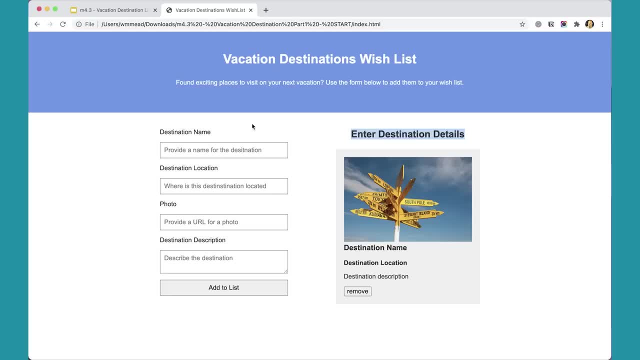 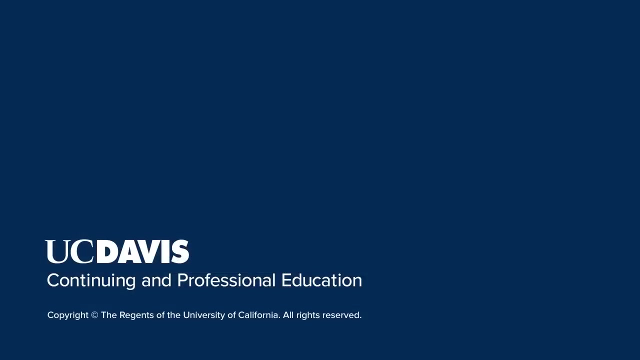 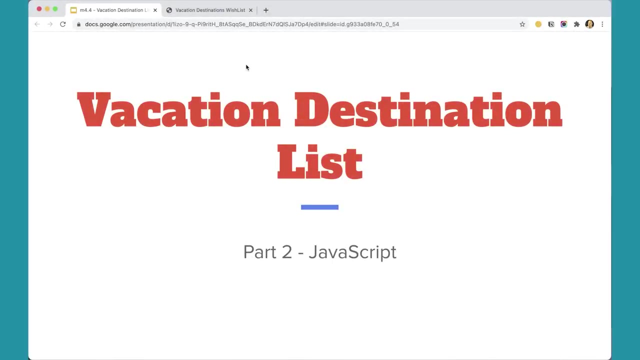 So I think it's worth taking the time to build the HTML and the CSS for this project So you understand what's going on and how the JavaScript is going to manipulate that HTML and CSS in the end to make the final product. Vacation destination list, part two. 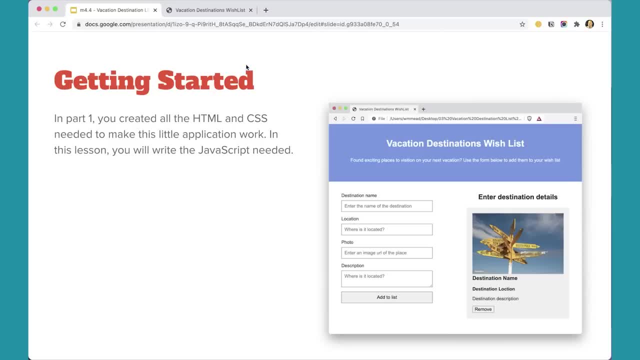 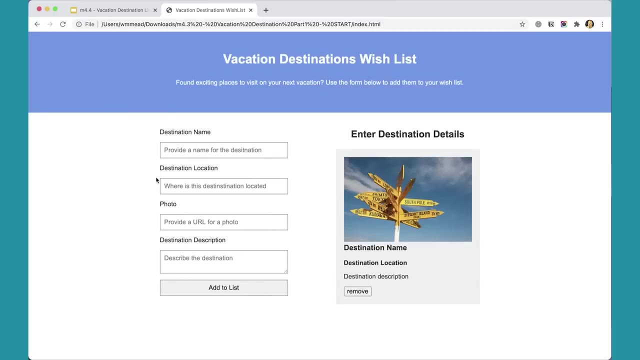 This part, we will add the JavaScript, and I'm picking up exactly where I left off after part one. In part one, you created the HTML and the CSS and you should have a page that looks like this. If you don't, please go back and make sure you go through everything to make sure that you get a page that looks like this before you start. 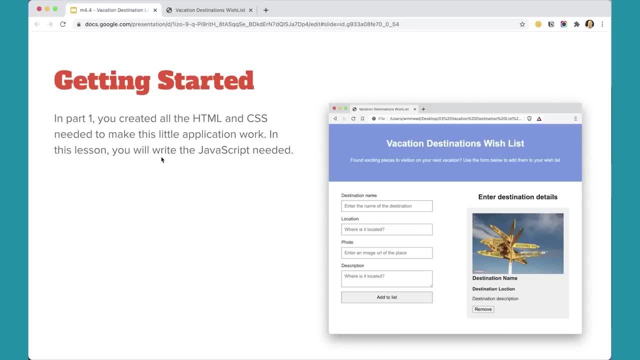 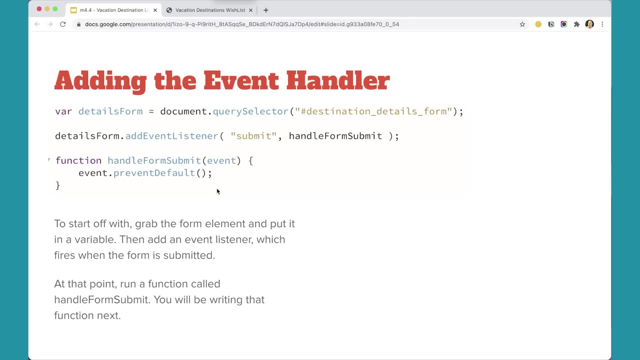 And you've got all the elements in there correctly. Okay, Everything's spelled right. Okay, So now we'll write the JavaScript we need to actually create this, make this little application work. To start with, let's grab the actual destination details form and put that into a variable called details form. 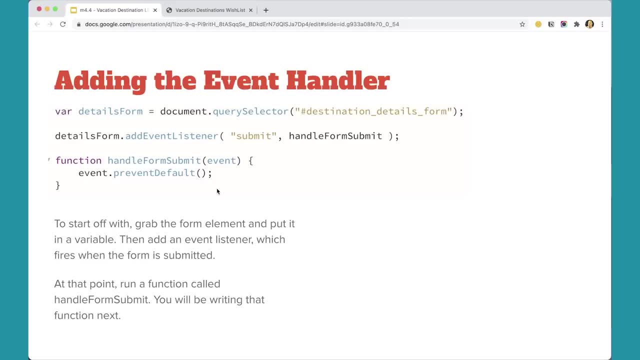 And then we'll have a event listener for when that form is submitted And instead of running an anonymous, we're actually going to run a named function called handle form submit And then we'll start writing the beginning of that function. So let's get started with this right off the bat. 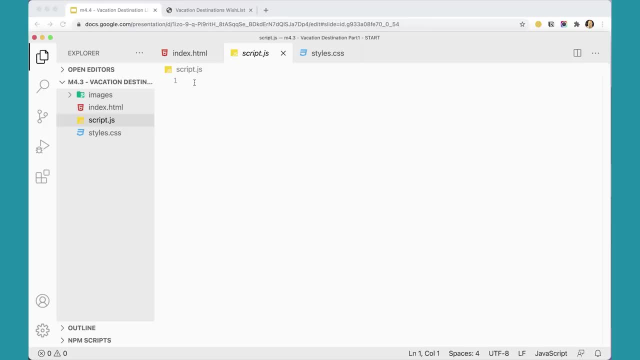 Over here I'm going to open up my script file and add a variable var destination. Yeah, I'm sorry, that's wrong. I'm going to do it. Details form equals document dot query selector. And I'm going to go get this pound details. 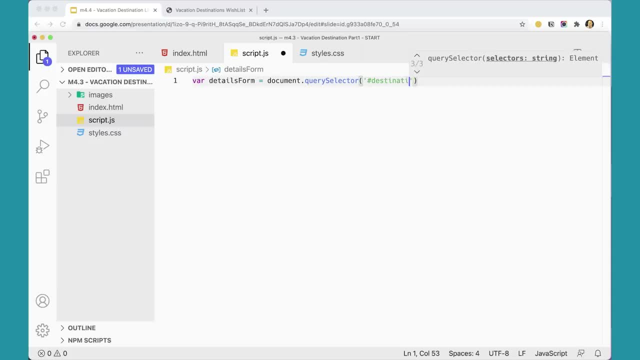 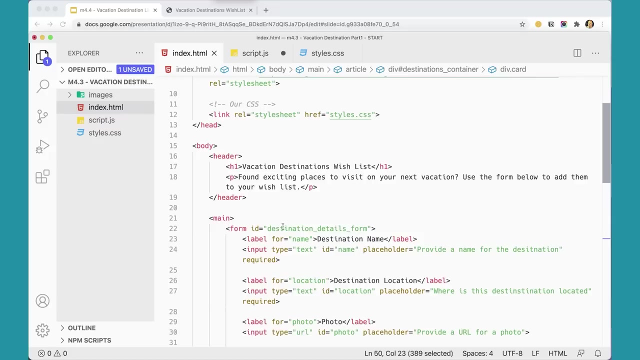 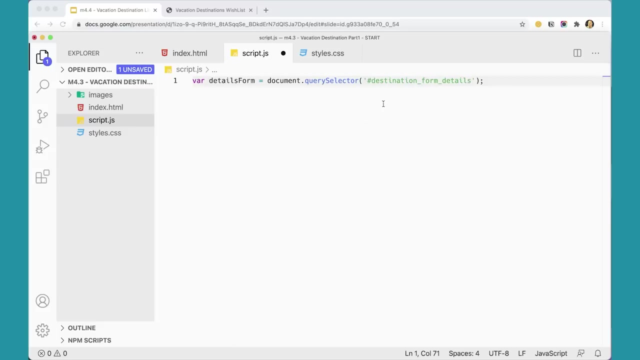 No, this one's destination form details. I think. Just check that really quickly here. Yeah, this form here, destination. In fact, if you want to be absolutely certain you spelled everything right, it's always a good idea, especially with these long names, to copy and paste that. 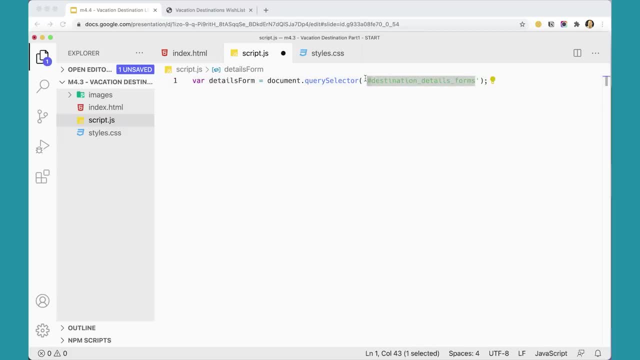 Note that I'm using a pound sign here because I'm using query selector. You could also use get element by ID, But that'll put this, That'll get that form and put it in here And that's great. So now we can do an event handler. 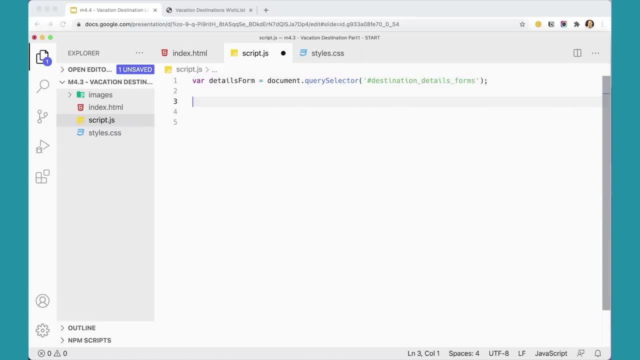 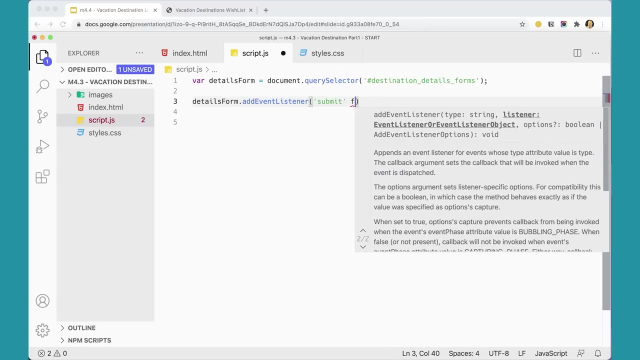 For details: form Details: form dot. add event listener And we're going to look for a submit event And then, instead of just doing function, like we've done in the past, I'm actually going to have a named function here called What did I call it over here? 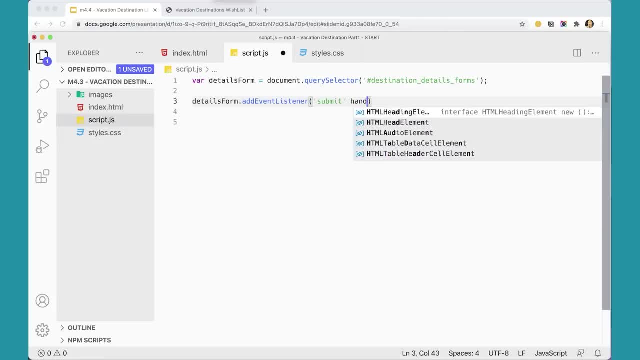 I called it handle form submit. So that's going to be a function that runs when this form is submitted. So now we need to define that function, function handle form submit, And this function we're going to pass in the event. object: Okay, 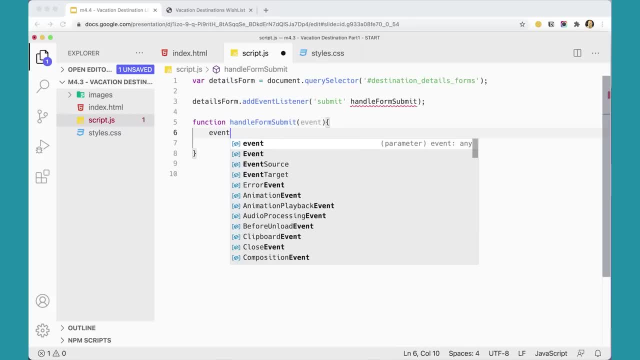 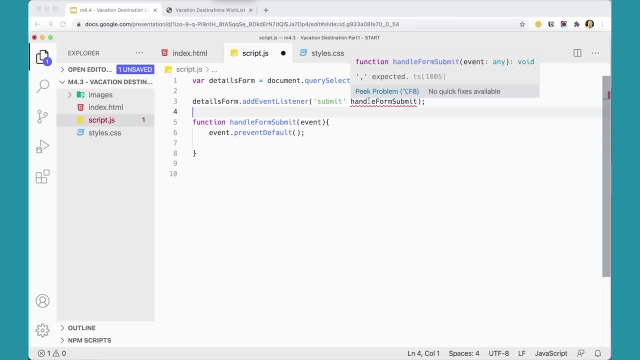 You might wonder why at this point, I've opted to create a named function here as opposed to just the inline function. And it could be an inline function. There's no reason why it couldn't. But this function, This function is actually going to do quite a number of things. 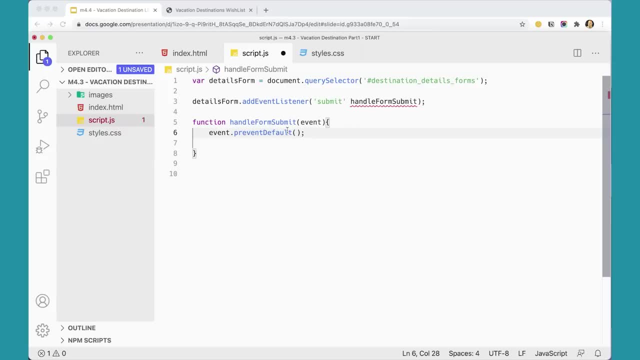 It's going to be a longer function. So I think it makes sense. I think it's a little bit easier to read in the long run if this is a separate function, since it's going to be a little bit longer. And that's just my own personal choice and my own style. 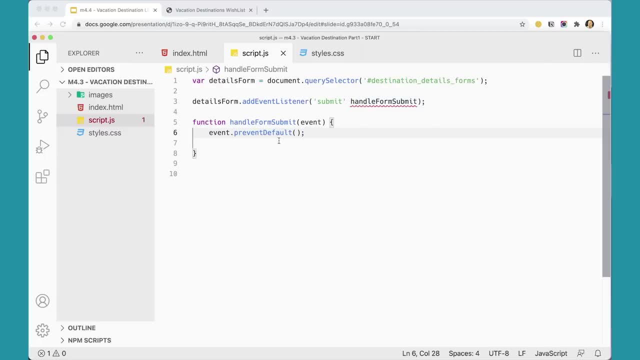 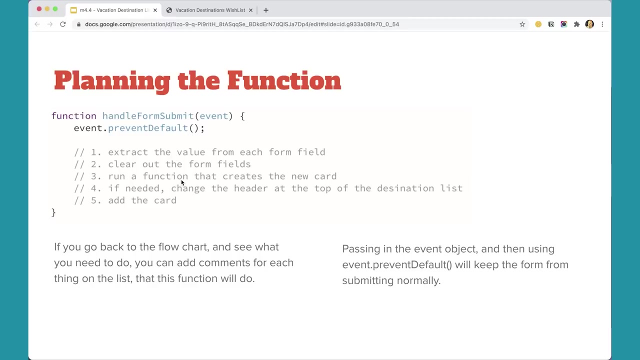 You could certainly use an anonymous function here and not have a named handle form submit function for this particular project. But that's what I kind of like, Because what we're going to do here, if we go back and look at this is this is going to extract out the value from each form field. 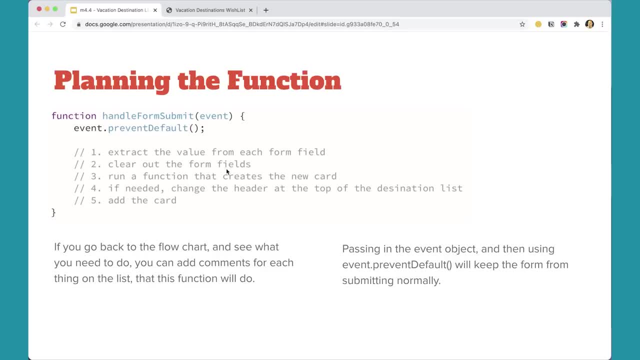 We're going to clear out all the form fields. So when you've filled in the form and submitted it, you need to clear out those form fields so that you're ready to make another card, And then we're going to run a function that creates the new card. 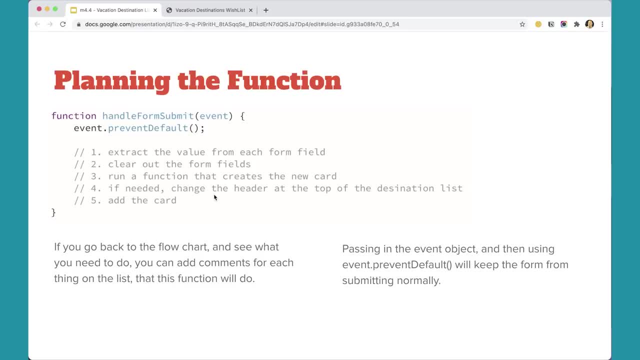 And then, if needed- meaning there's not already a card over on the right-hand side of the interface- we need to change the header at the top of that destination And then actually add the card and you can go back to the flow chart from the previous, from the previous version of this, from from part one, and actually see how that's going to all come together in the flow chart there. 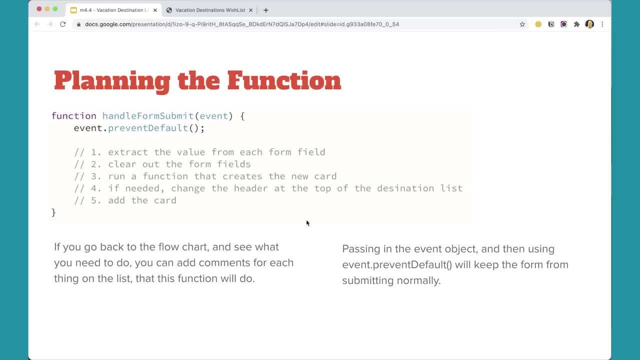 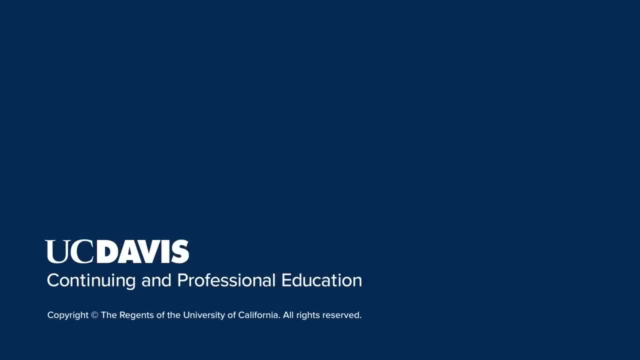 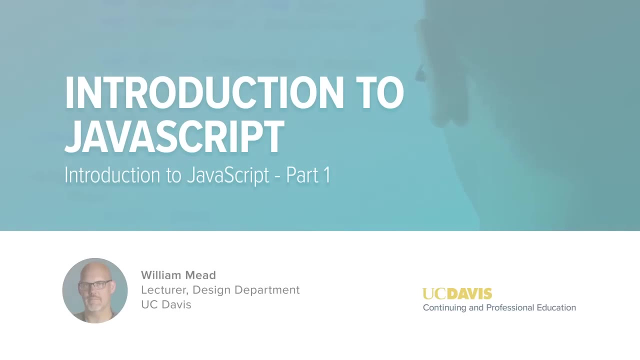 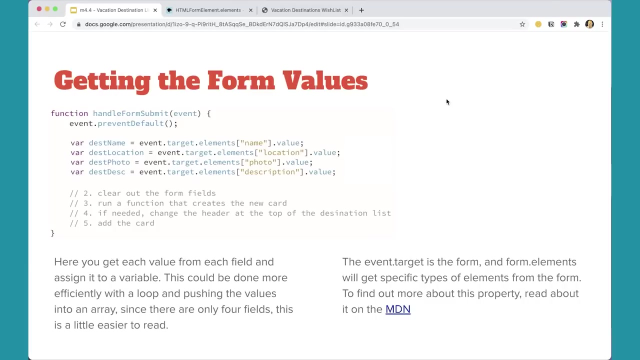 So yeah, so we start with event prevent default to keep the normal submission of the of the form from happening. But then we're going to do all of these Things. The first thing on our list of tasks to do is to get the values out of the fields from the form. 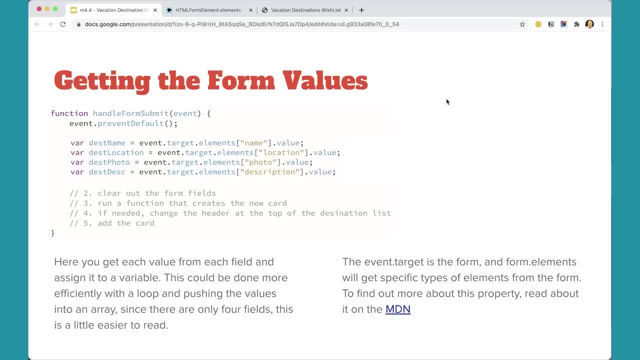 And to do that we can create a variable for each of the four form fields- the name, the location, the photo and the description- and then go and get them And then we're going to get the value out of those from that, from that from the actual form. 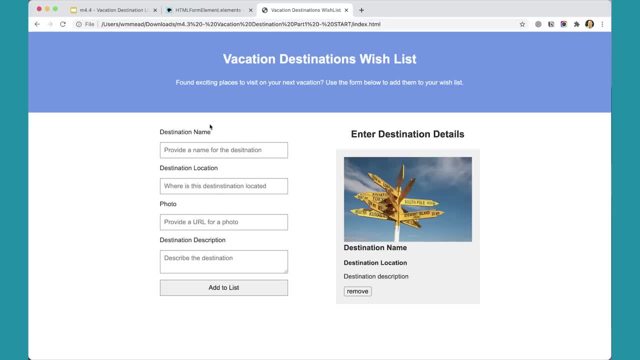 And you'll remember over here, when we created this form, in the HTML we made it such that these fields were required. So if you try to click add list without filling in anything, it's not going to. it's not going to do anything because of that required thing, at least if you're using Chrome or a modern browser and we can get more into form validation and making sure you get. 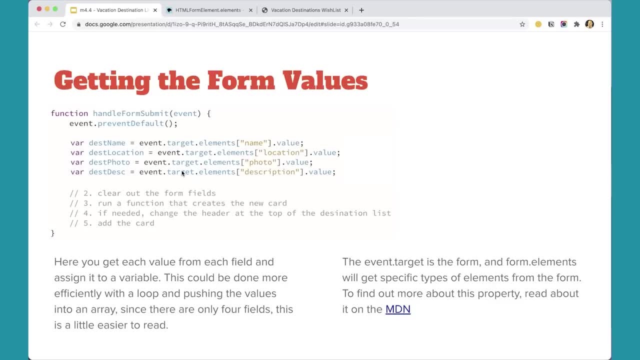 Good data into forms in the second course in the specialization. But for right now we just want to. we just want to do something quick and simple and we've got enough there to sort of keep it from at least being empty, even though we're not doing very much for that. 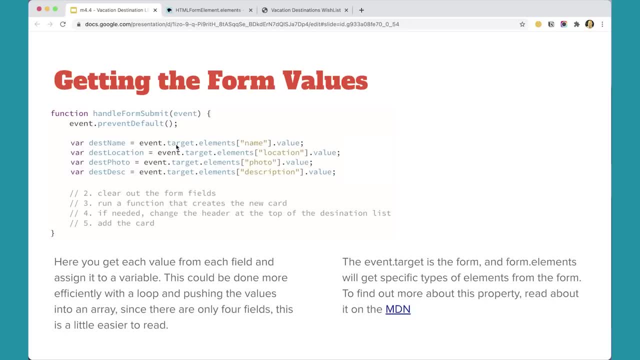 And what we're going to use here is we're going to use event. event target will be the form submission right, because that's the, that's the event target, or the form itself, And then we can get the Elements property and pull out each one of these elements out of the form and its value and put them into a variable here. 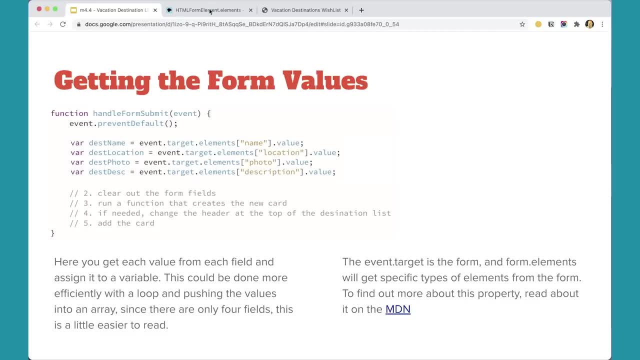 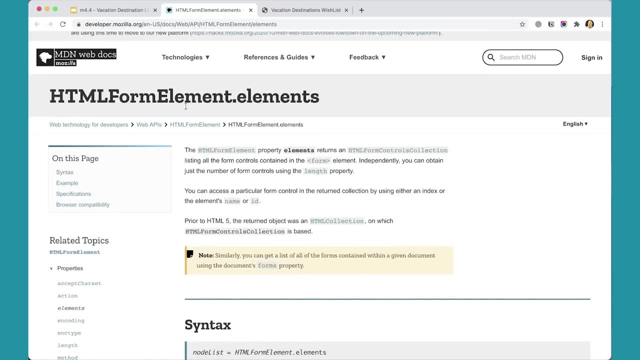 This target dot elements is something you know. the dot elements refers specifically to form elements and you can come over to the MDM and look at HTML form elements, dot elements- and find out more about what this is, But it'll get you a specific. 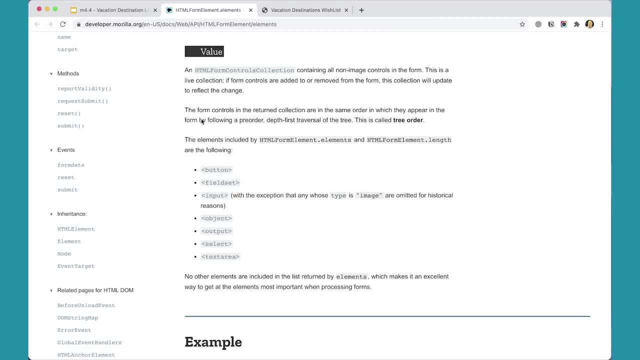 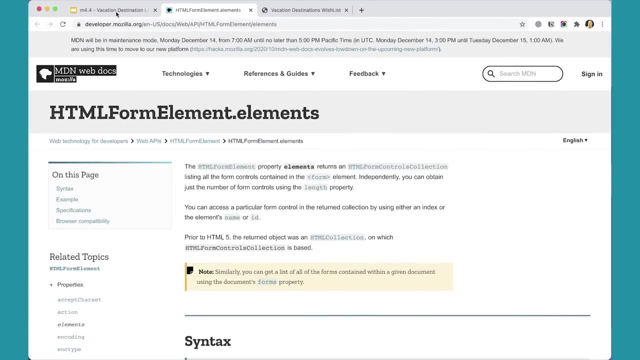 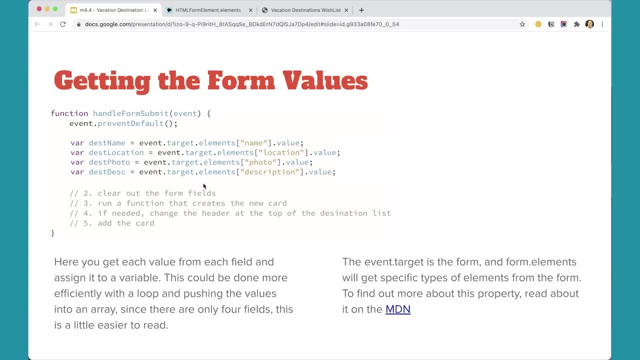 Set of elements specifically from forms, And so it's kind of a helpful little property here that we can use to get specific elements out of out of the form and get that data. So let's go ahead and put that on to our script. So over here I'm going to do. 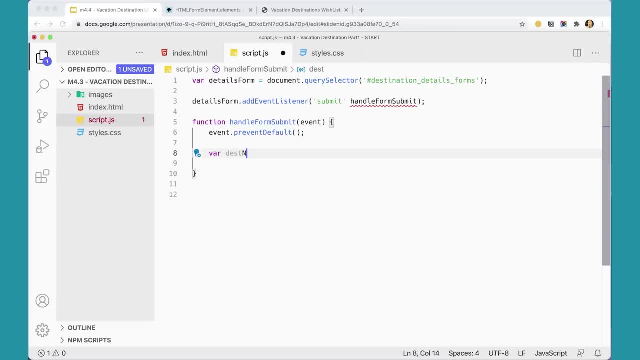 Our desk. Nation name Equals Event dot. target Dot. elements, Square bracket. Because which element am I going to get? Name? That'll get me the first one And I can just copy this And paste it. Destination Location. if I could select this. 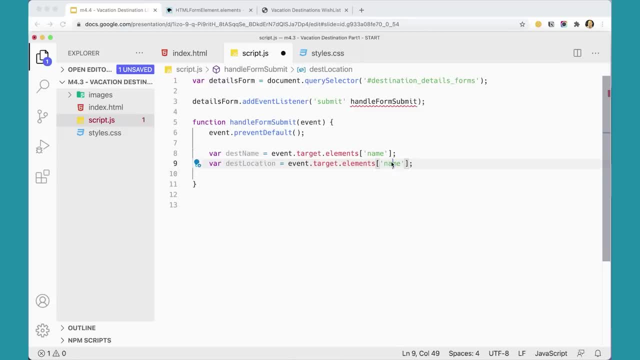 Destination Location is going to be the location field, And then I'm going to paste again Destination Photo Is going to be the photo field, and then paste one more time and then we've got destination description, which is going to be the description field. 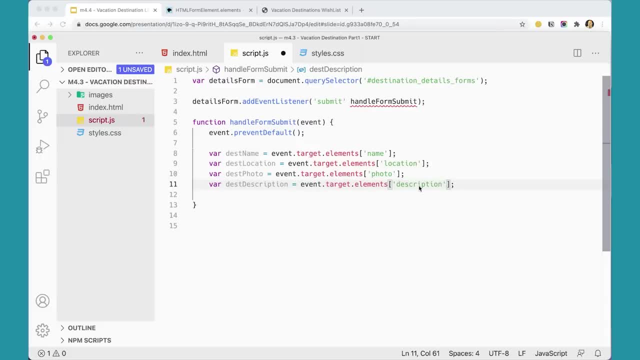 actually, i'm going to short this down, short this down to esc and then- don't forget, i forgot this already- we need to get the value, so we need to add dot value to each of these, and this one here, too, should have done that initially, but there we go. so that's going to do the first part. that's going. 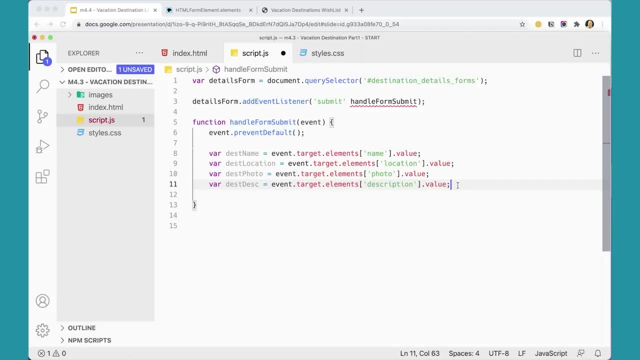 to go in and into our form when it's submitted, submitted, and get the value of our eliv in the beginning. so that's going to do that, and then we get the the values out of those fields that somebody typed in and put them into these variables here. 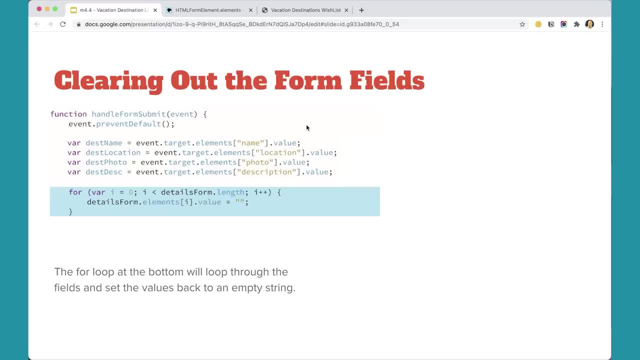 The next thing we need to do in our list of things to do once we've captured the values from the form, is to remove them so that the form is ready for a new thing. So I'm just going to use a for loop here to loop through the elements of the form and set the value. 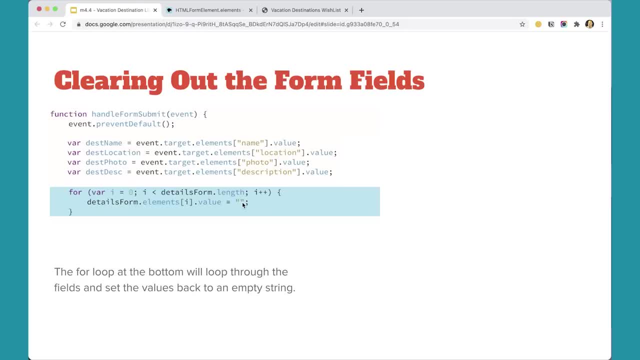 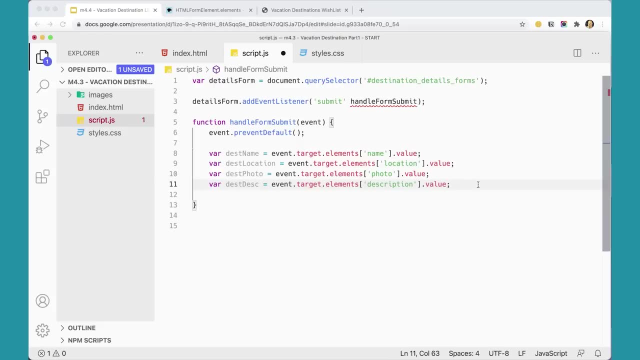 back to empty. And here you can see I've got just quote, quote. I'm setting it back to empty, So let's go ahead and add this next as the next thing this function needs to do here. For here's my for loop, for, and I'm going to have just a counter variable: var i equals. 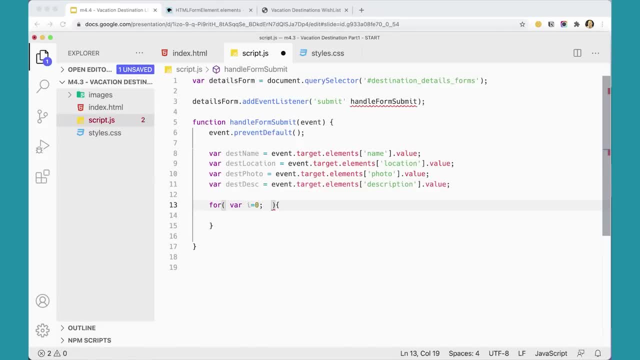 var i equals zero. well, i is less than details form dot length. there we go. oh, details form dot length: i plus, plus, there we go. so that loop is going to go through details form and remember details form is going to get everything inside of details form there, and and then what I can do in here is I can very easily 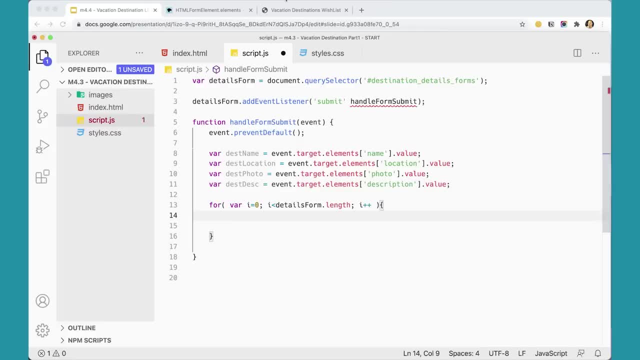 say, okay, details form- dot elements, square bracket. i dot value equals quote. so we're going to go through the details form and i starts at zero. and the first first time through the form it's going to say: okay, get element zero from that form and set its value to empty. and then we're going to increment i from 0 to 1 and if 1, if there's more. 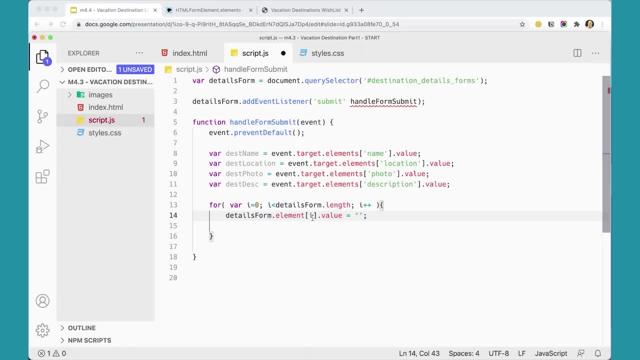 than one element in the form, then we're going to go through and do that again for element one, setting it to zero, setting its value to zero, and we're going to do that for each element in the form until the form is completely cleared out. so that's just a very simple for loop, that's. 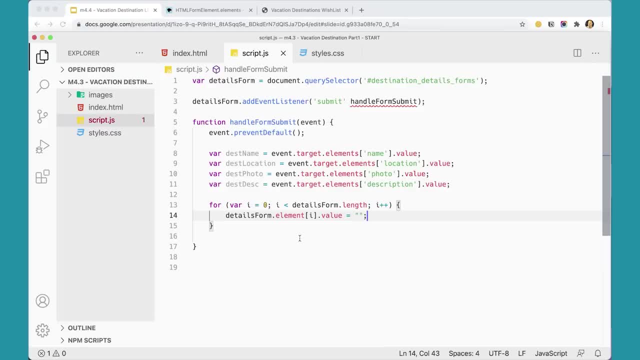 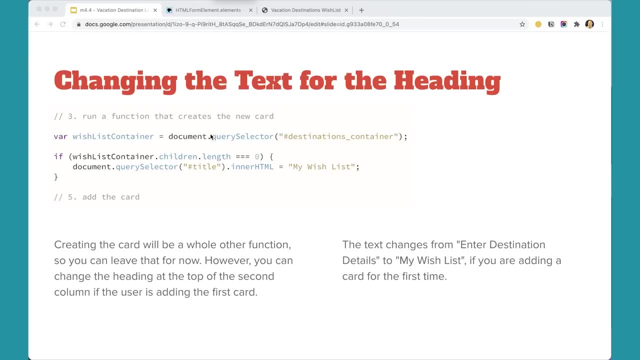 going to loop through and clear out each of the elements. in that form, we've taken care of the first two items on our list. we gathered the information from the form and cleared the form out. the third thing to do is to run a function that creates a new card. 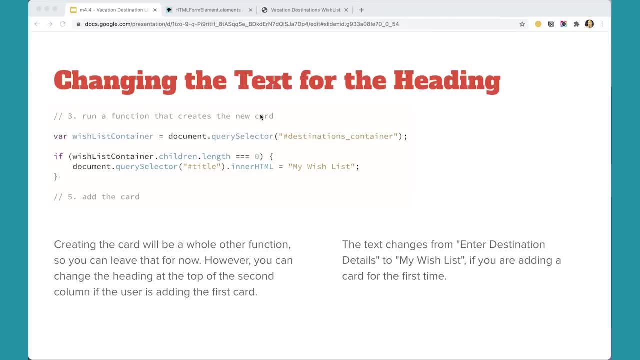 and we're going to hold off on that. so we need to write that function. but we can take care of the fourth thing, which is to check to see if we already have a card in the other side and if we, if we do- do one thing and if we don't, we won't, uh, we'll do a different thing. so 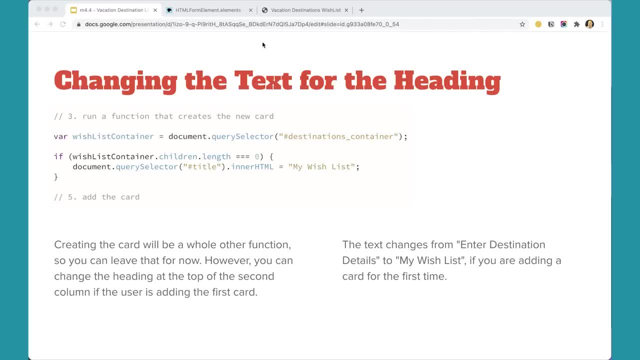 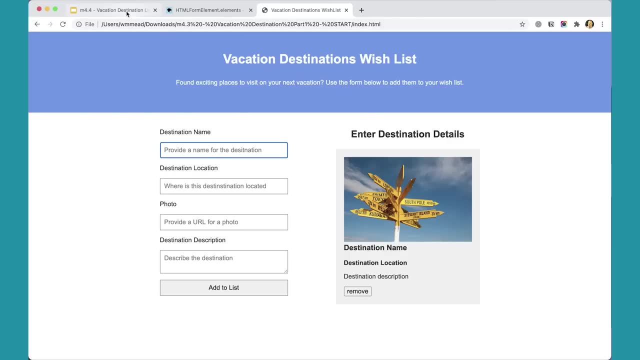 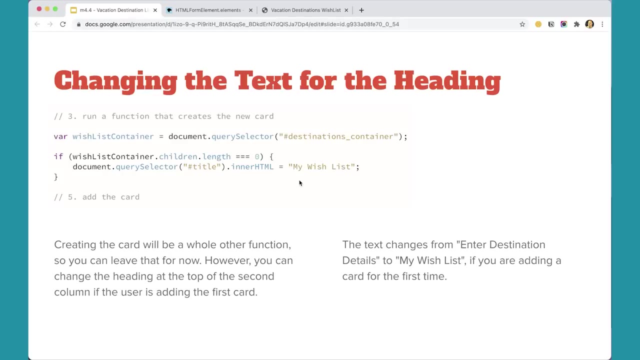 we can take care of that in terms of the header over there and in showing and determining what this header says here. either it's going to say enter destination details or we're going to change it so that it has something like my wish list in there, because that makes a little bit more sense once there's something in. 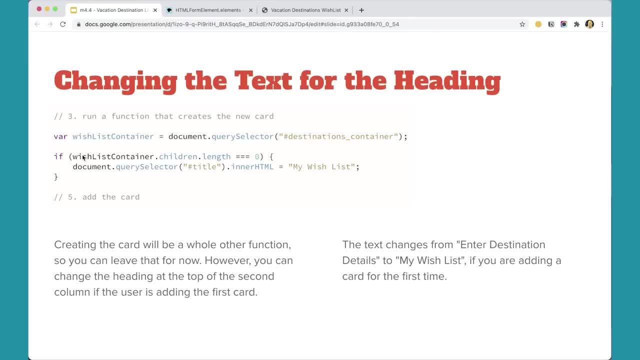 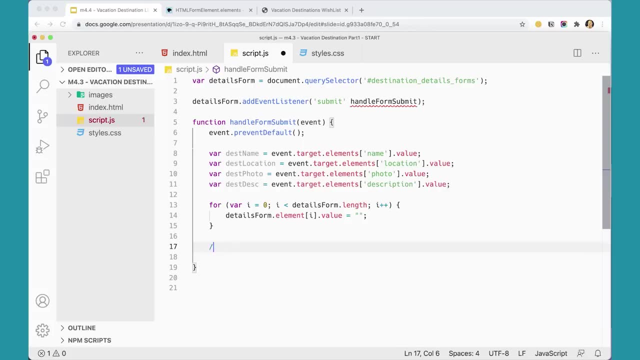 in that column over there. so let's do that really quickly. we're going to make a variable. we'll just put in add, create password here so we remember we need to come back and do that. but i'm going to have var wish list. container equals document. dot. get element by id. 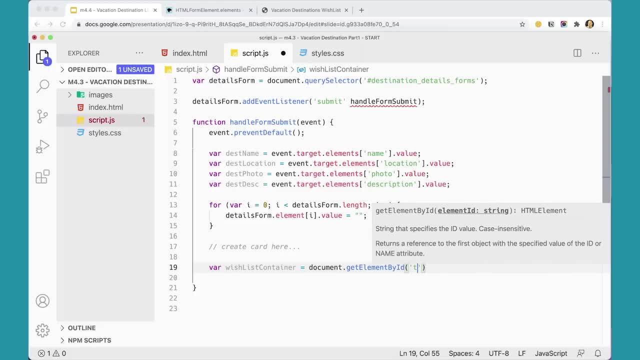 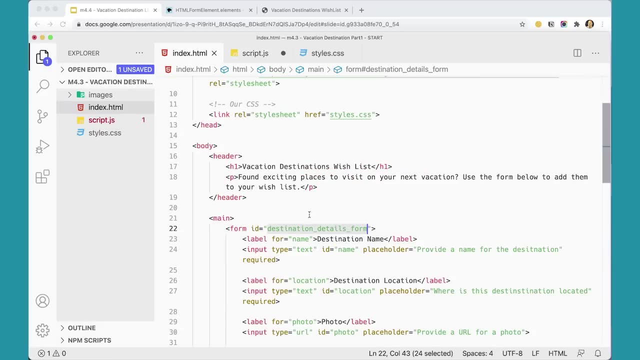 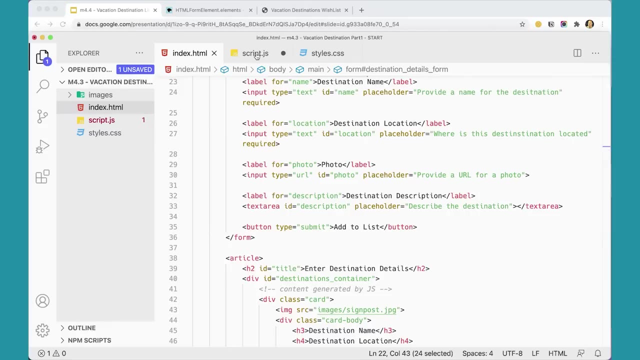 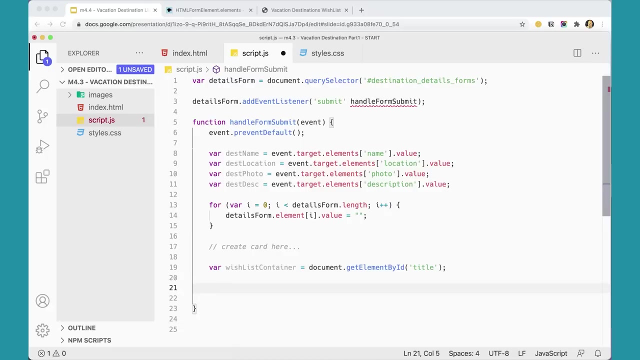 and you'll remember we have, say, junk. you should remember when subject and 5 are from when and what had an id called title specifically so that we could do this over here in the html. you'll remember we have down here title on that id. so get element by id title and then we just need to see. we just need a little if statement here. if 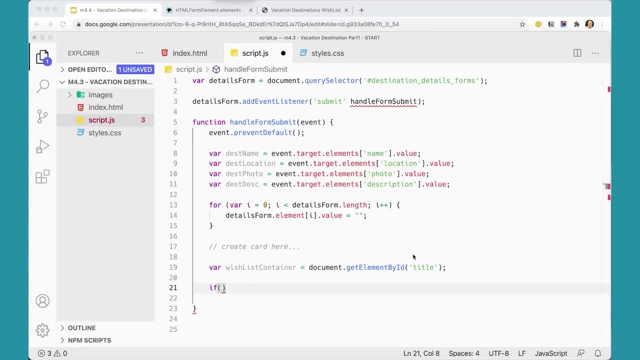 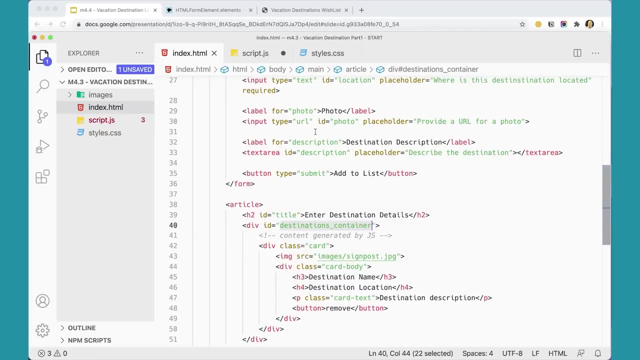 oh, whoops, i'm realizing i did the wrong thing here. i don't want the title here. i want to get the um, this id down here, this destination container, that's the thing i want to check for: destination container. i want to see if, because i want to see if we'll do the title in a minute, but if. wish list. 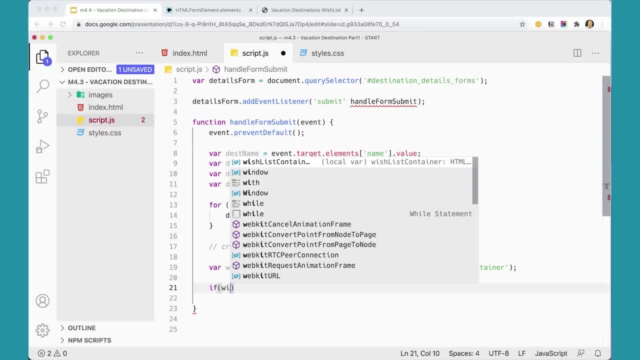 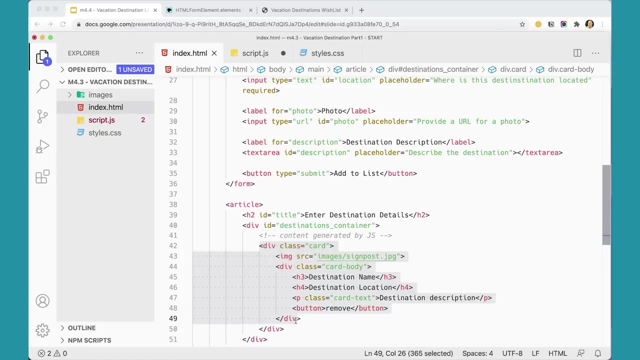 container. i want to see if we'll do the title in a minute, but if wish list dot, children dot length is exactly the same as zero. so if there's nothing in this container and over here we've added a card in here temporarily, we're going to get rid of that. but if this container is empty, 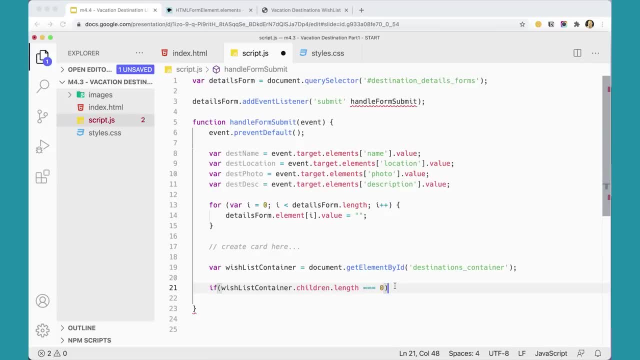 then we're going to do something. if it's empty, then we're going to say, okay, document dot. get element by id. now we want the title. it's inner html is going to be: what did i put in there? quote my wish list. there we go, and that will take care of the fourth thing, which is: 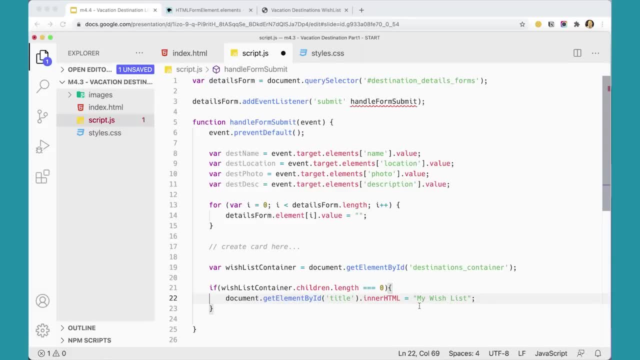 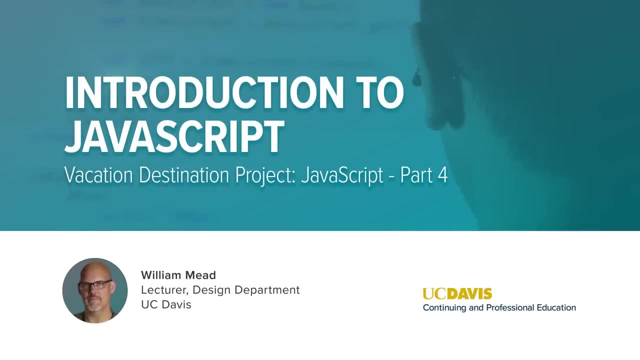 if we haven't added a card in there before, it'll change the title over on the right hand side there. behavior over here. it gets the data from the data agent and then over there we'll rule by item. so we'll create an item and we'll add it to the div. you give them data from the topic. the tree that happened to be the cord was so caught-up over here. we'll do this as a default and try and implement the math problem in a couple of ways in a moment with an update. if we're going to put a combination product, some parts of it but packed with that and this one don't work, but it works i mechanism of behavior. it gets the data from the control computer. so what we're going to do is define certain parameters and choose what so it can be applied. 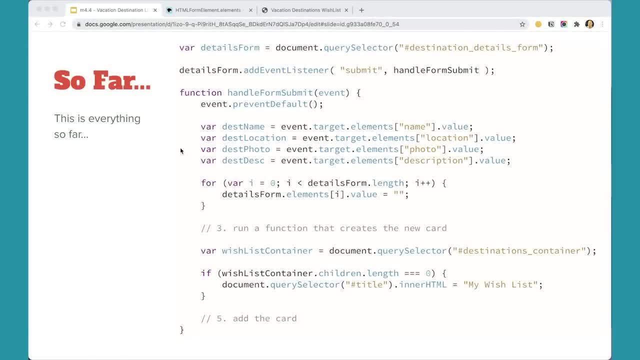 gets the data from the form fields and then clears them out. We have a placeholder for a place where the function that creates a new card is going to go, And we're going to write that next. And then we check and see if the header on the right-hand side of the page already 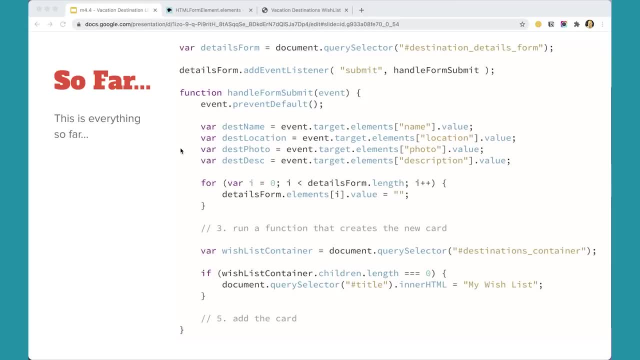 if there's already a card in there or not, And if there isn't, we're going to change the text inside that header over there, And then, finally, the last thing that we'll do is actually add the card. So let's move on here. 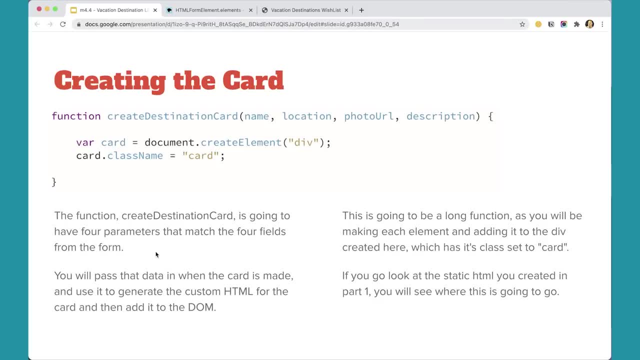 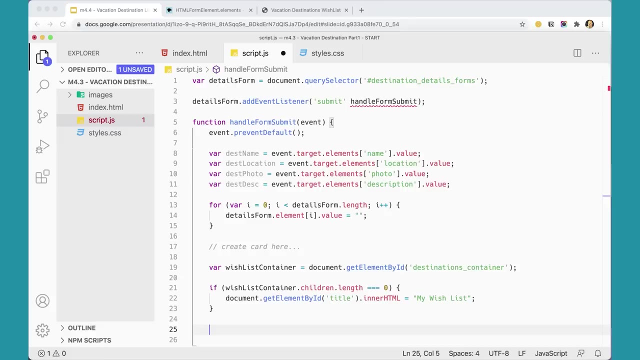 We're going to create a new function called createDestinationCard, And it's going to take four parameters, And these parameters are the data that come in from the form that somebody filled out. So let's go ahead and do that first. So down here I'm going to create a new function. 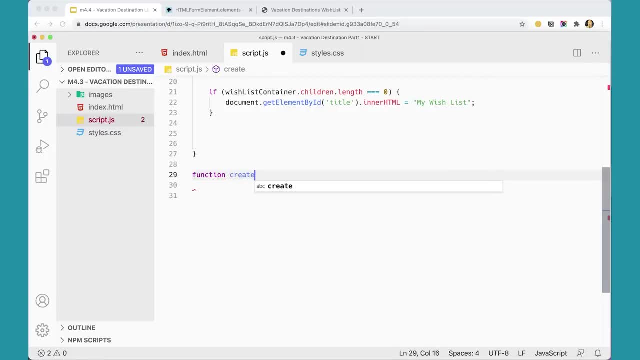 Function, create DestinationCard, And it's going to take name, location, photo. I think I just did DESC for description. It's going to take those as parameters, Although they don't get quotes on them: Name, location, photo and description. 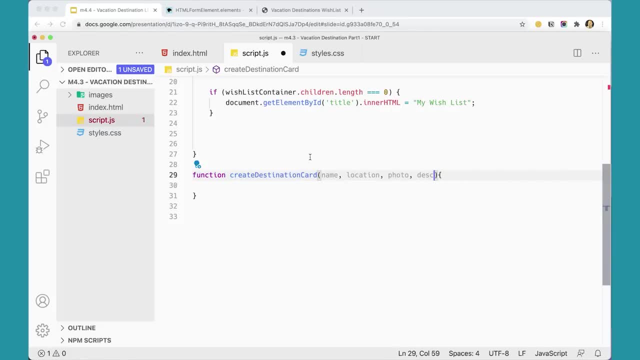 That's right, Okay, good, So we're going to pass those variables in. Actually, I'm going to change. I'm going to change this a little bit. I'm going to actually make this photo URL And I'm going to type out description over here. 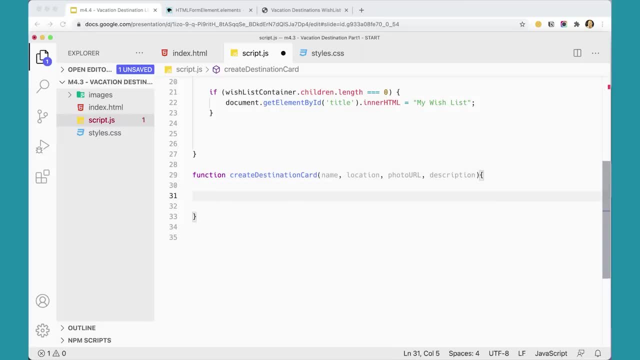 There we go, And then I need to make var card And this is going to be assigned documentcreateElement. We're going to create a div And then we're going to take that card and we're going to set the class name equal to card, I think. 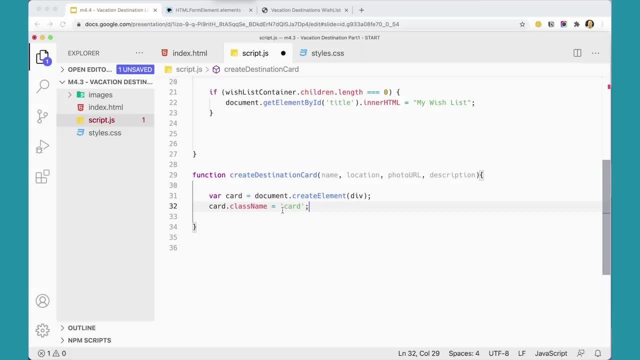 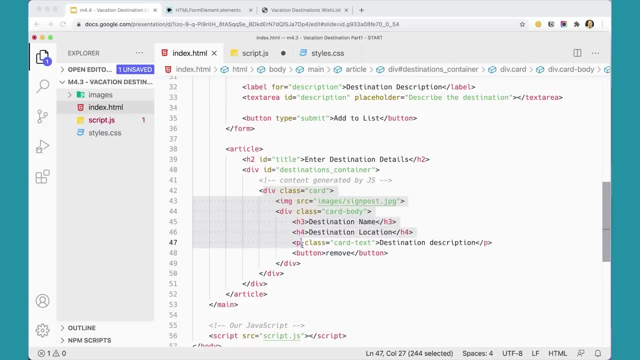 Yeah, card. And if you wonder where we're going here, you can go over to the index file here, Because we're basically going to use JavaScript to create these elements And put them in the card. So now we've just created this div here and given it the class of card. 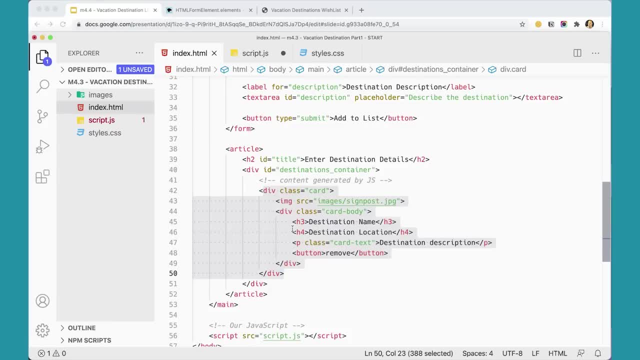 So that's what we've done, And this is going to be a long function Because we have to create each one of these elements individually And put the content in them and then add them to the card, But it's not that long. 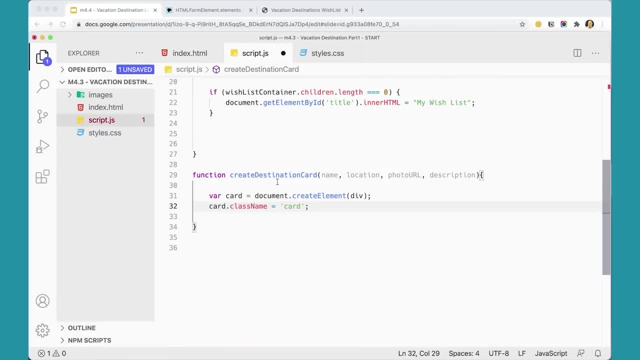 But it's kind of useful to see how this is going to work. All right, so we've got that. Next we're going to add the image. So first thing we need to do is make a var called img Or image or whatever you want to call it here. 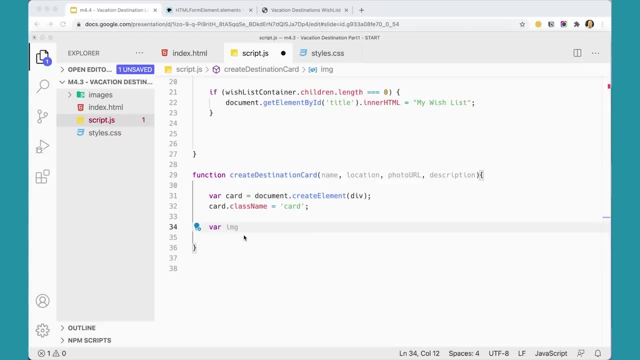 I'm just going to call it img And then from there I'm going to do equals documentcreateElement, And we're going to create an img element And then Images really should have an alt attribute, So I'm going to say imgattribute. 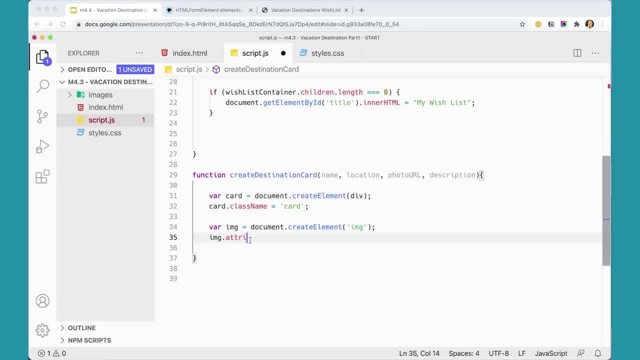 Now, what do I want to do here? No, it's set attribute. That's what I need. Set Whoops, that's not set. Set attribute Alt, And I'm just going to set it to name. So whatever gets passed in as the name of this location is going to get set as the attribute for the alt tag. 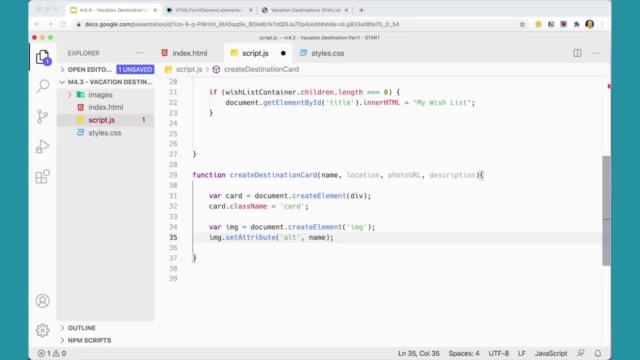 So if somebody is using a screen reader, they will still be able to know what it's a picture of, Even if they can't see the picture. If they've got a visual disability of some sort or another, Okay great, So we've got. 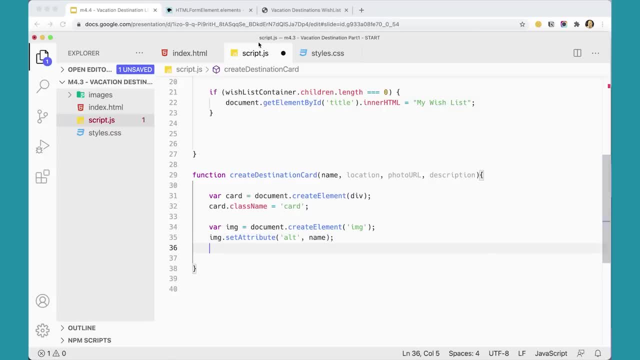 We're setting that attribute, We also need to set- We need to set- the source based on what comes in through this photo URL here. So we want to be able to set that photo source, But the photo source is not required. So the first thing we need to do is determine whether or not a photo has been brought in. 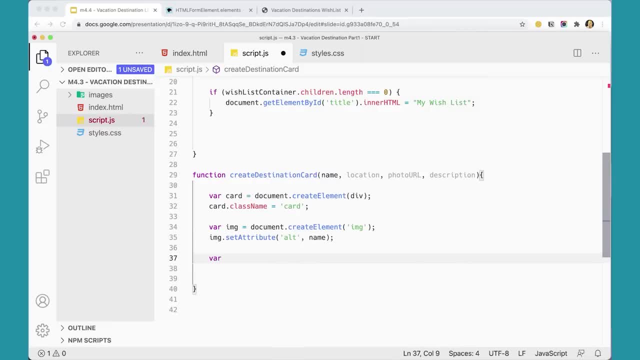 And before that we want to just make a variable Var And I think I call this Constant Photo URL And I'm going to make that equal to Images Slash Signpost JPEG, Because that's the image that's in this folder over here. 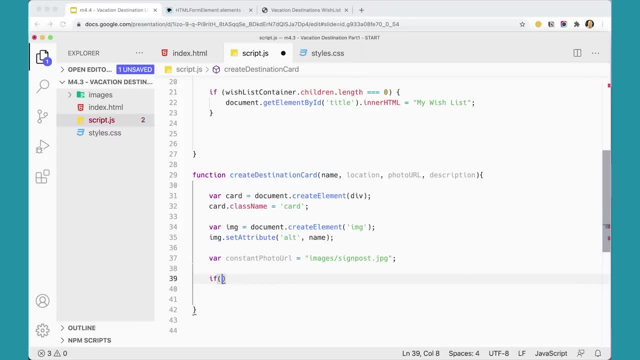 So then I just need To see if Photo URL- That variable there that gets passed in- Did somebody actually add a URL in there. And we know that it has to be URL in there because over here in our form we set this to type URL. 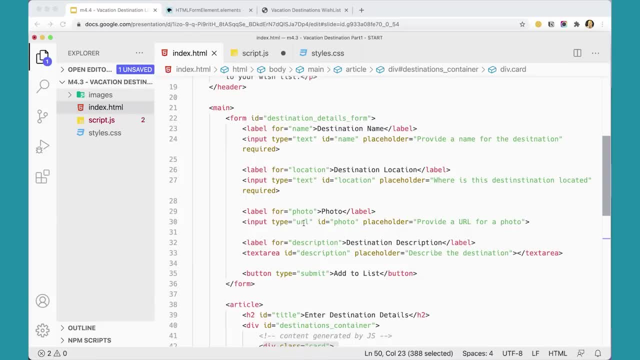 So it'll only take a URL, Otherwise you'll you'll get a Chrome barking at you and telling you that you didn't put it in a A URL. So we put a URL in there and if one actually got put in cause, it's optional. 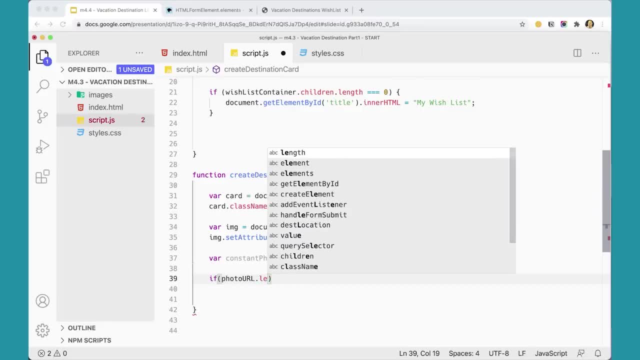 Um. so if photo URL dot length is Greater than zero, I think that's what I'm doing. No, actually I want to check and see if it's exactly the same as zero. If it's exactly the same as zero, then what I want to do is I want to set the um, set the image. 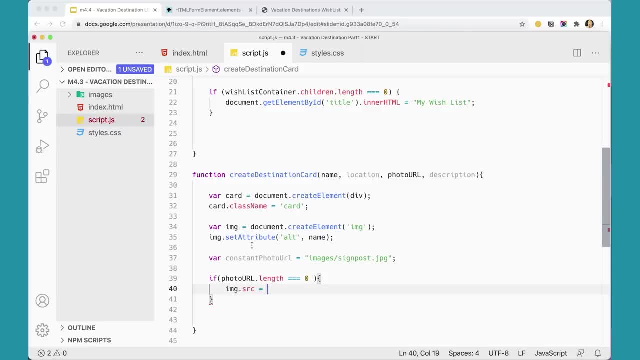 To SRC equal to this constant photo here. I'm going to set it to that. I'm going to set the image source to that. That should work. on my slide I use set attribute again, So maybe I'll do that just to make sure, but really this should actually work just fine. 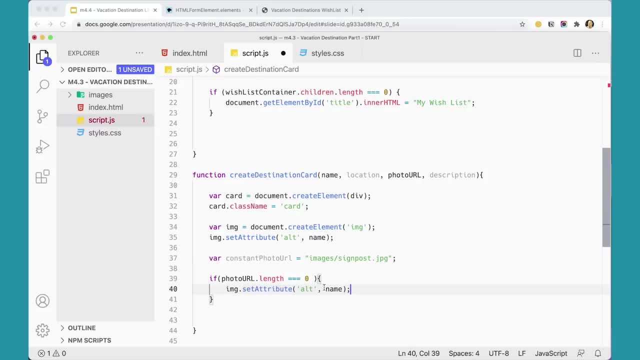 Um, but let me just put this in just so it matches what I'm doing on my slide there. So attribute SRC is going to be this constant photo here, constant photo URL, And If that Length isn't exactly zero, zero, the else will be okay. 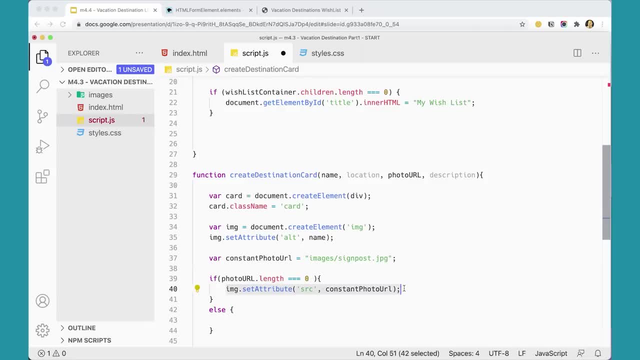 We're going to, uh, do image set attribute to not constant, not for this source there, but we're going to set it to photo URL. So if somebody put in a URL for a photo it will get set to that. Otherwise we'll use the default one that's in there. 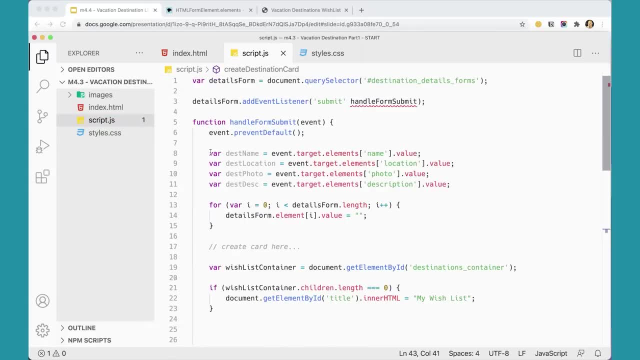 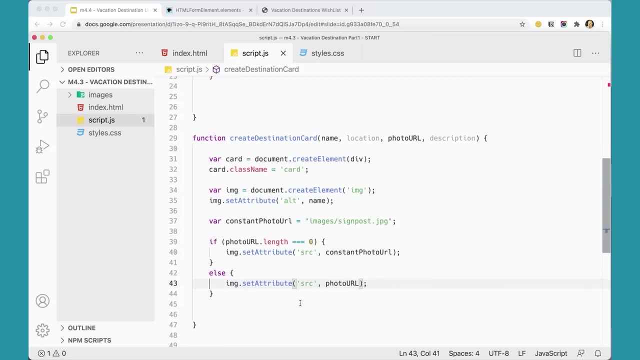 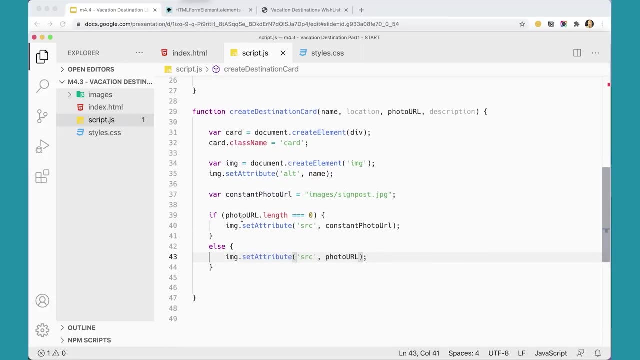 And this is unhappy about something here. I'm sure what I've done wrong. Sure, It'll come up sooner or later. Okay, So I'm not quite ready to test this yet, even though I'm picking up. there's an error on my script somewhere, but we'll find it in a minute here. 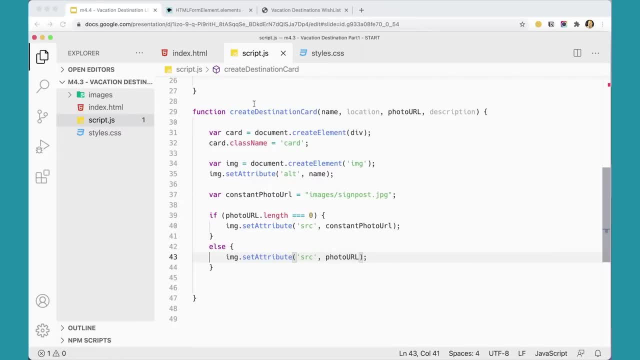 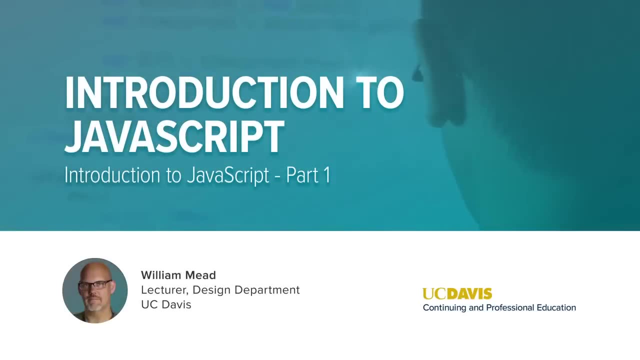 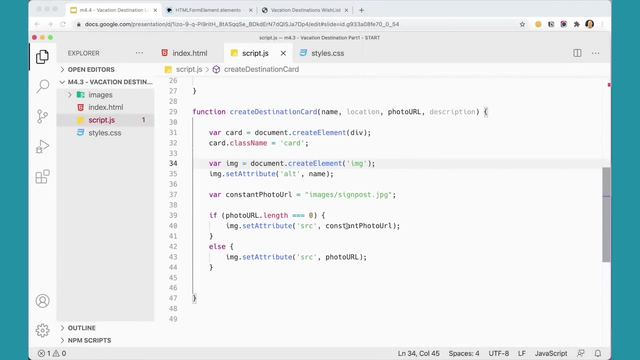 But, uh, this should, this should work for now And then we'll pick this up in the next video. This function is getting long and it's going to get longer because we're creating all of these elements here. So if you look over here on the index file, what we've created so far of our cards, we've created this div and we've created the image. 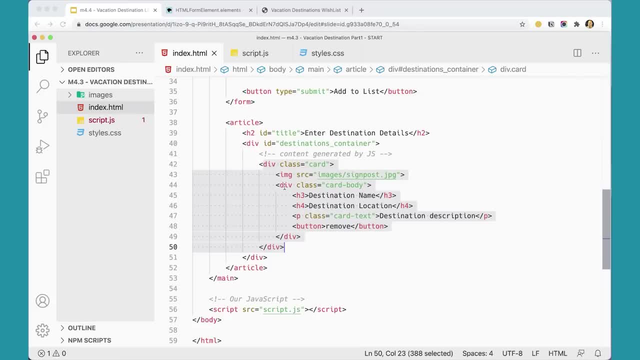 Next, we need to create this div for the card body And then add into that the H3,, the H4, and then the description text. We're going to add all the numbers here. Okay, the description text is actually optional. if you come up here, you'll. 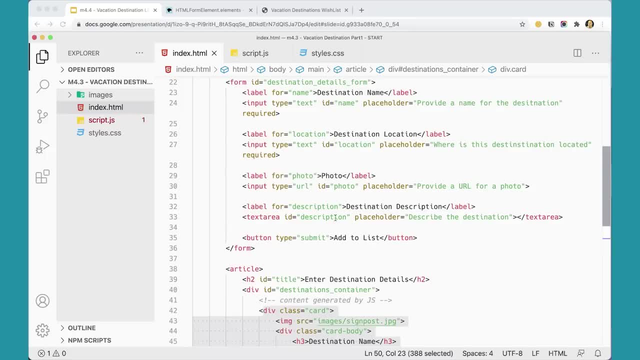 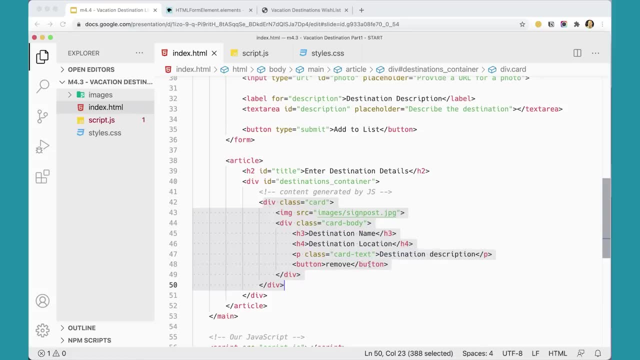 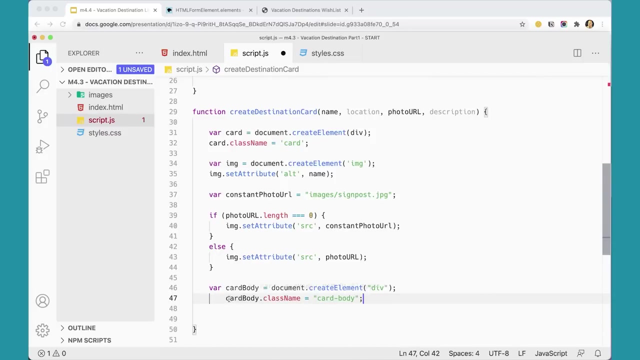 notice. there's no required on the text area there, so we're gonna have to deal with what happens if that's empty as well, and then we'll have to add the remove button as well. but let's go ahead and continue forward with this. so over here. the next thing we need to add after the image is a variable for the card. 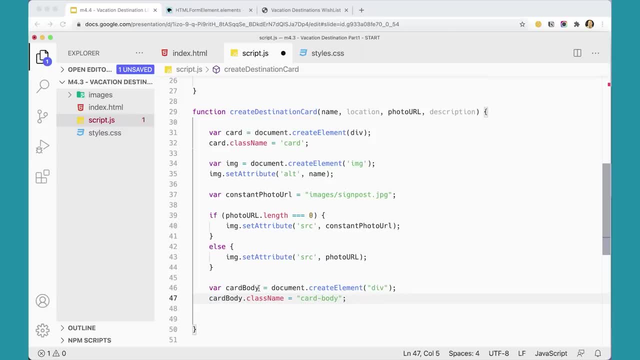 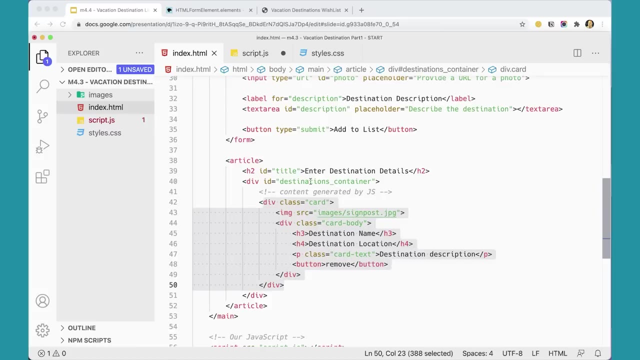 body that's going to. we're going to make a variable card body and create element div and then set the class name to card body for that and that will create that card body element here and then next we need to do the same with the h3 and the. 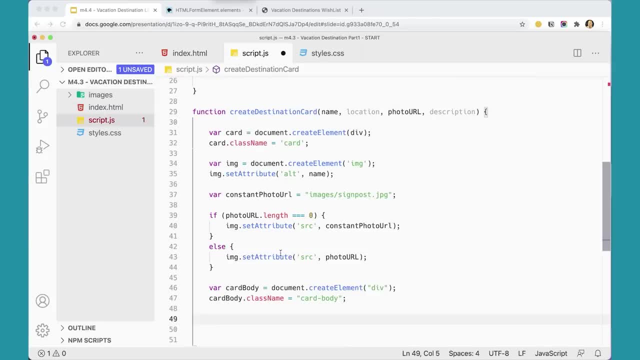 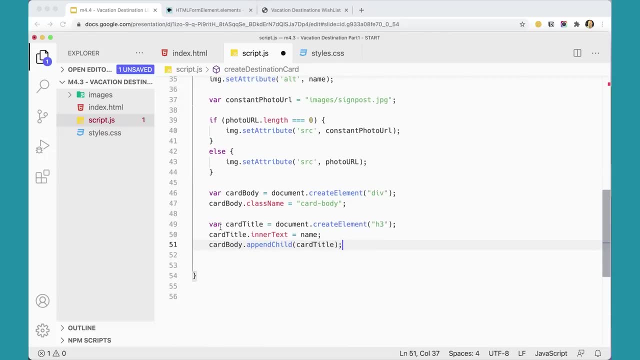 h4. here's the h3 and I'm just going to paste it in. you'll have to type it, but i made var card title document get a create element h3. so i've created an h3 and then i'm setting the inner text to the name again. this is the name. 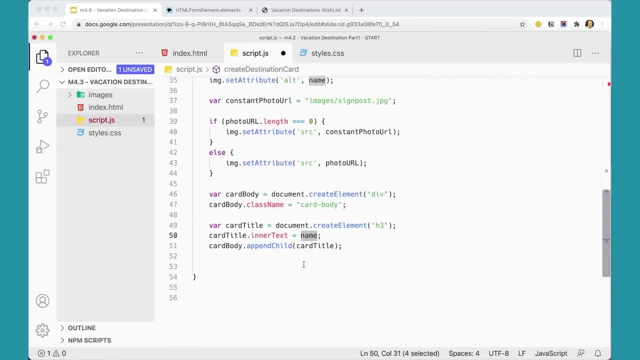 that came through from the form. that's what's going to get put in there. so that's going to be the name, and then i'm going to append card body. i'm going to append child card title. so i'm putting the actual card title into the card body here, and then we'll do the same thing with the. 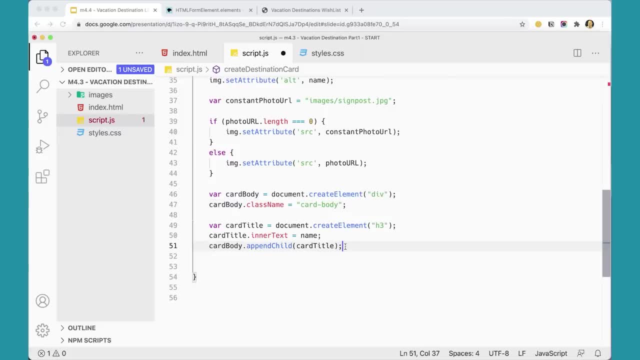 subtitle. okay, so now i can add in the subtitle- and again i'm going to paste this in so you don't have to watch me type it, because that's getting kind of painful for everybody. but i'm going to make a variable card subtitle and create element h4 and then i'm going to set the inner text to: 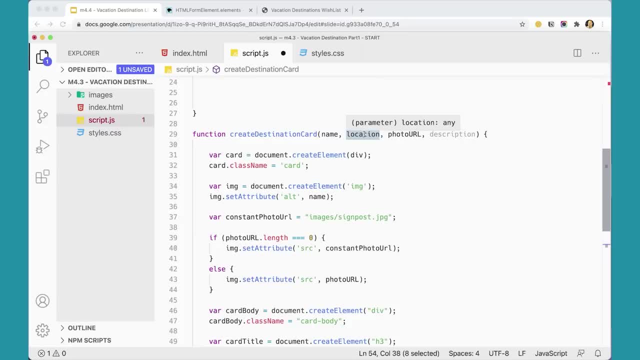 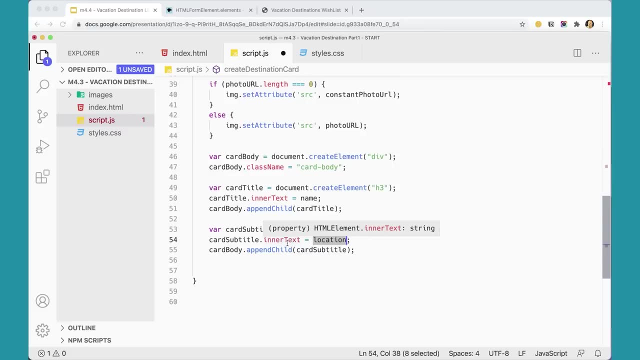 the location. so that's this location that's getting passed in here, that's the location that somebody typed in on the form and so that's what that's going to get set for the inner text there. and then i'm taking card body and i'm appending the child. 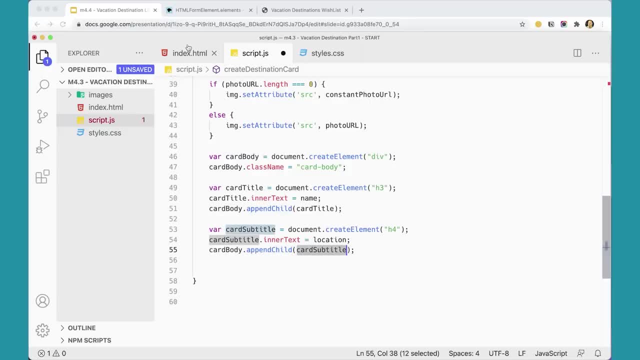 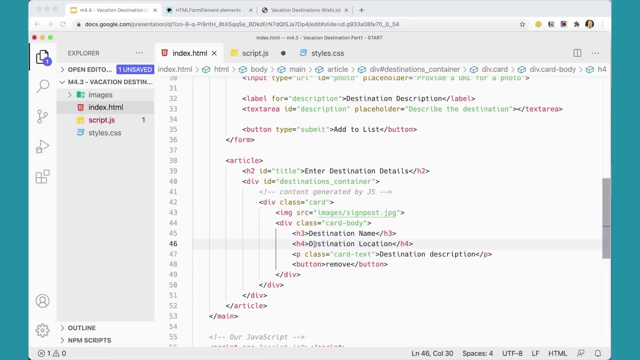 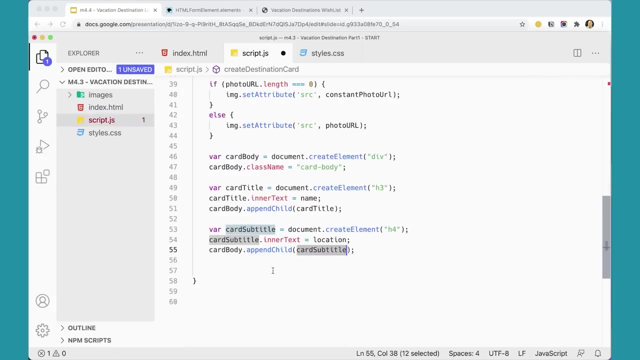 card subtitle, so that that's going to add this to the card. so i'm appending that in there. so i've got card body and i've appended in the h3 and the h4. next step you is to check and see if somebody types something into the description, because it could be empty potentially. 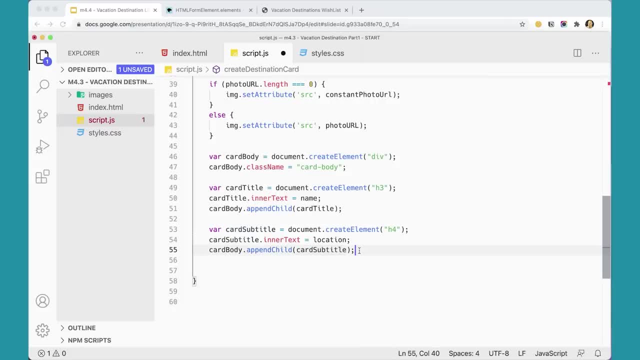 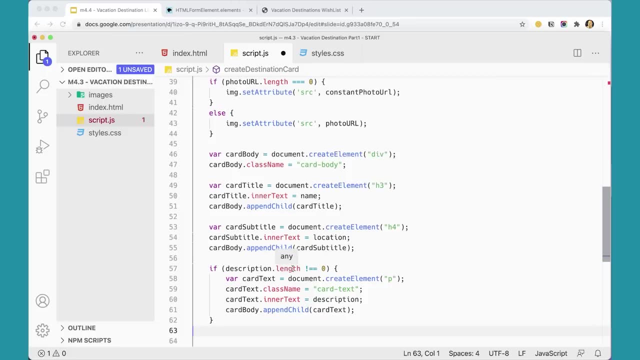 And we'll put that in next. Again, I'm going to piece this in so that I know that it's right. But here we go. If descriptionlength is not 0, meaning it's longer than nothing, then we're going to make a variable cardText. 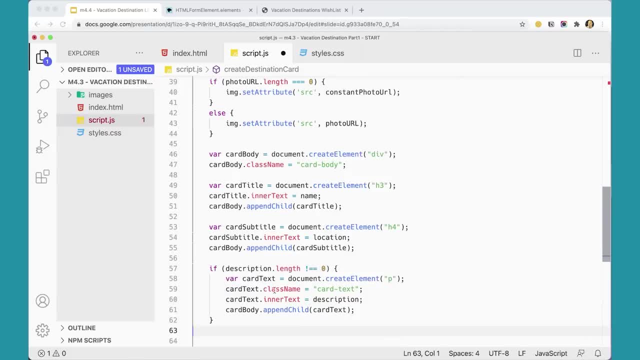 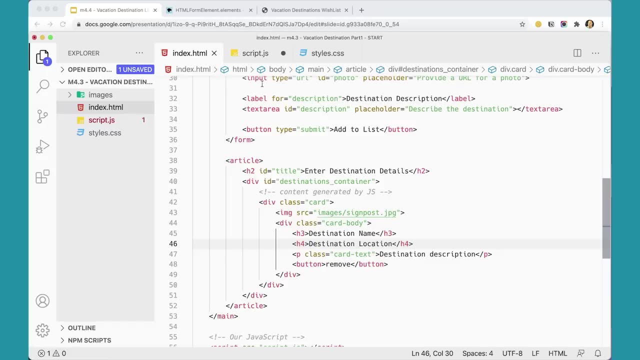 and create a paragraph And then we're going to take the class name and set it to cardText Because again over here- remember we did that- We have p class cardText, So I'm setting that class name in there to cardText. 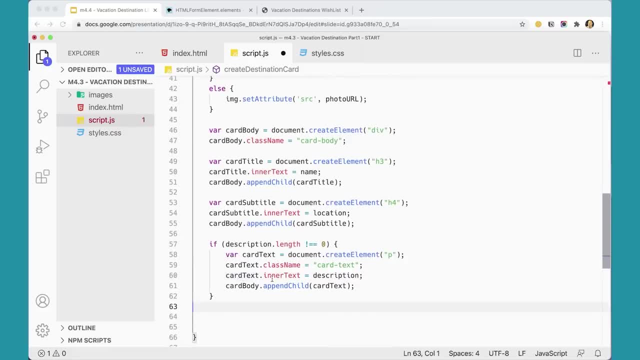 so we could style it specifically if we wanted to, And then setting the innerHTML to description and then appending that cardText to the card text And then setting the innerHTML to body again, so we get that appended in. The next thing we need to add is the remove button. 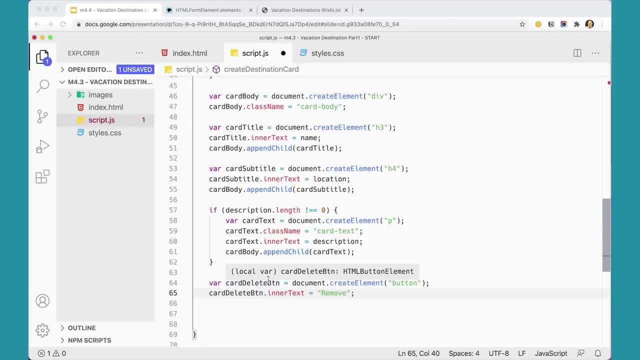 So we'll put that in here. So here I've got a variable called cardDeleteButton and I'm creating a button And I'm setting the inner text to remove And that will create that button and set the text for it to remove. 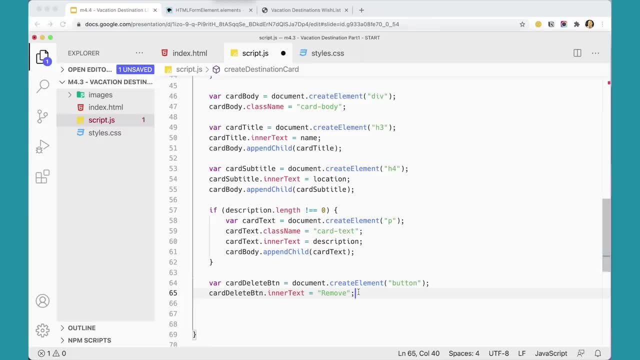 And then I need to add an event listener. I'm going to add an event listener, So that button is going to create an event listener And I'm going to add an event listener called remove destination. We'll write another little function that will actually 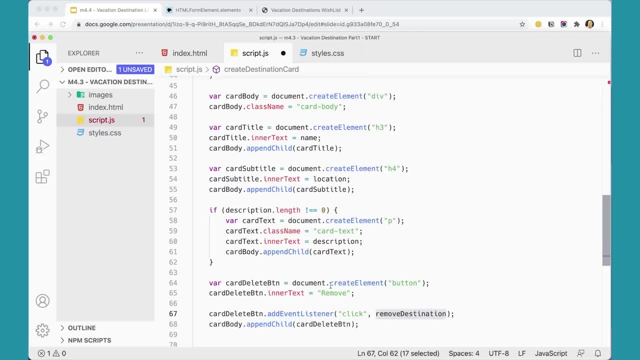 remove this destination. But I'm putting an event listener on this button right now, as soon as I add it, And it's going to have its own event listener. that's going to run a function And then I take that card, that button, and I'm going to add it. 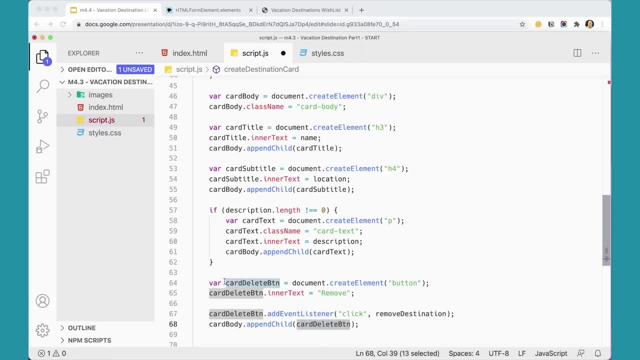 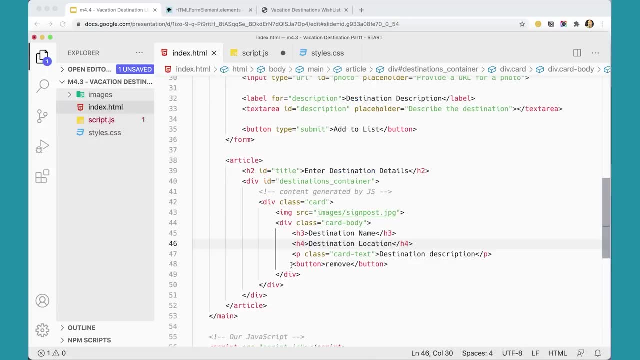 I'm going to add an event listener to this button And I append it. I append the card delete button to the card body. So again, if we come over and look at the HTML here, you can see that this button called remove has been added. 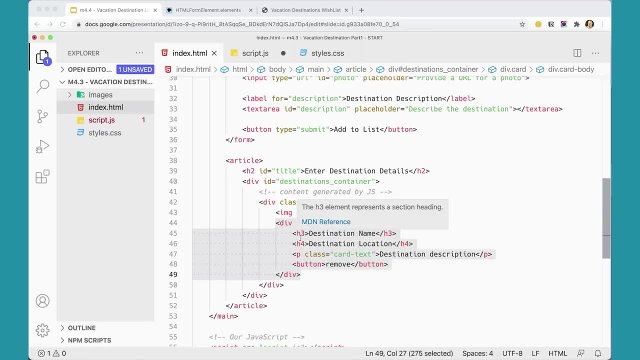 to this card body. So the card body includes four items: the h3, the h4, the paragraph and the button. It only includes the paragraph if somebody typed something in that field, But it includes the button, And the button has an event listener on it. 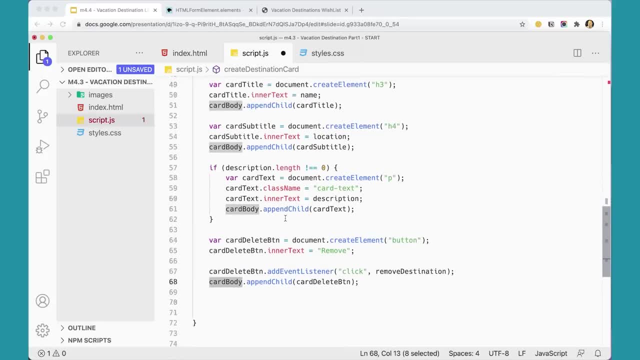 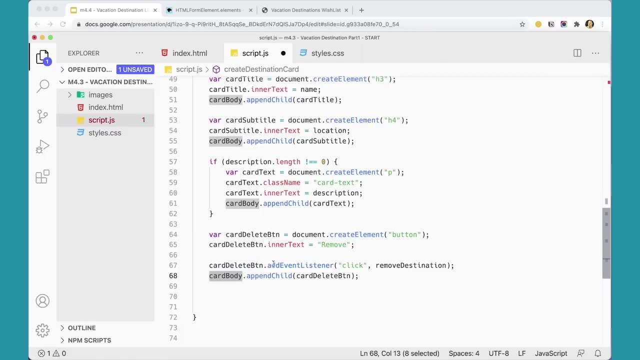 That will run a function that we haven't written yet, But it's there, OK. So that's going to put all of those things on there. Now the next thing we need to do is take this card. We've been building up this card body. 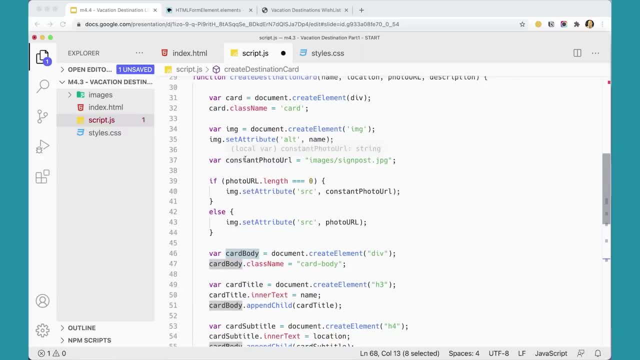 So we need to take this whole card body and add it to the card, Because we added the image to the card. We created the image And we set its attribute And we set its photo. Maybe we didn't add that to the card? 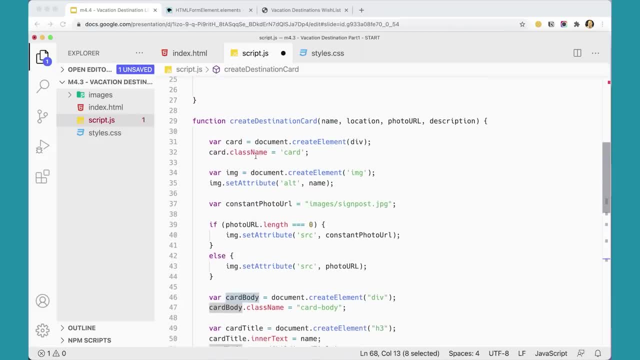 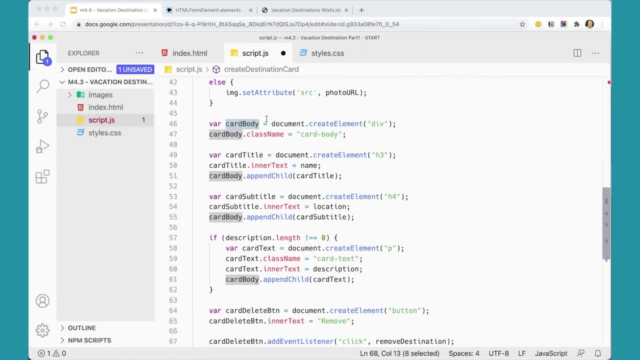 We need to do that too. And then we created the card. Yeah, We need to add the image to the card as well, But we need to add the card body to the card too, Since I forgot to add the image, let's do that first. 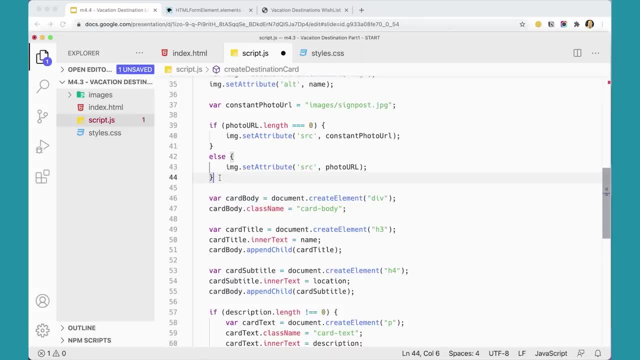 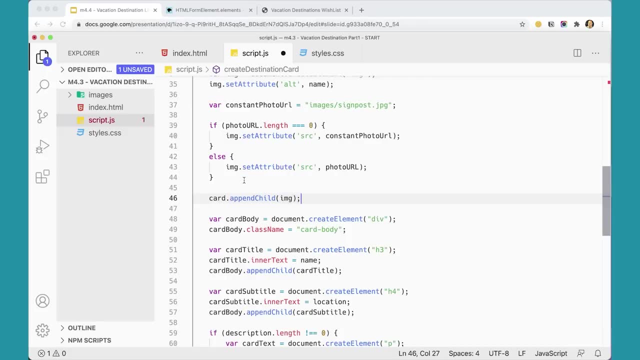 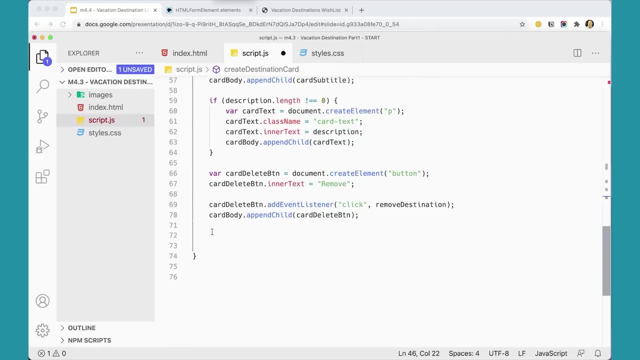 So here we've done the image. We've got the image all in place. In here we need to add card append child image, So that will put the image on the card And then down at the bottom here we need to add card append child card body. 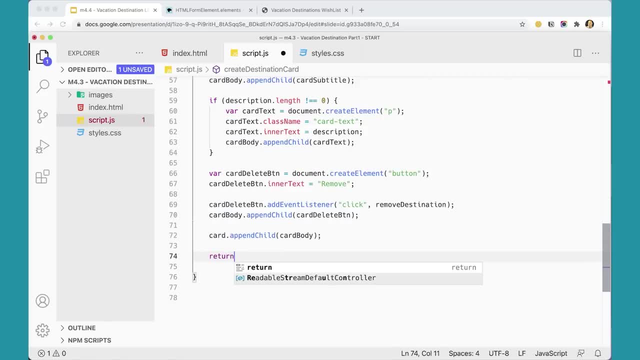 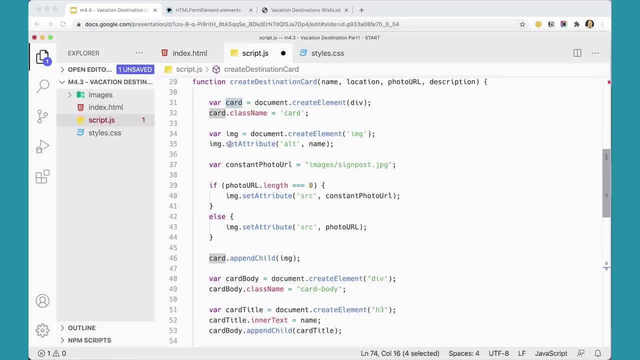 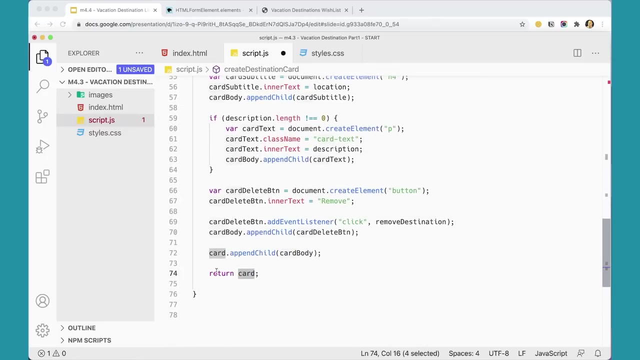 And then we just need to return card. So that's going to take this card object, Or this piece of HTML that we've created that has all this stuff in it, and return it. Okay, So this is a long function that makes all of these elements and returns that card, which should be a big piece of HTML. 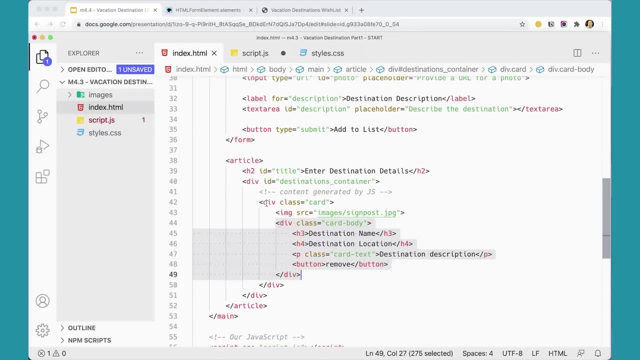 Well, not a very big piece of HTML, but a piece of HTML. that's this card here, div class card, And in it we'll have the image, either the signpost image or one that somebody entered a div called card body, and an h3 and h4, possibly a paragraph, if somebody typed one in. 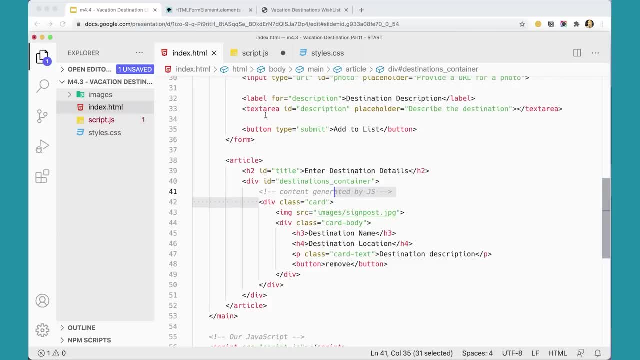 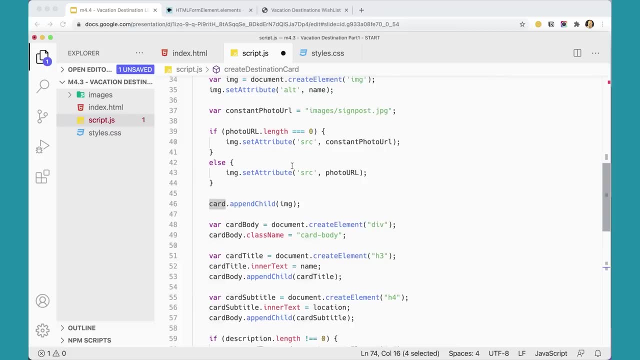 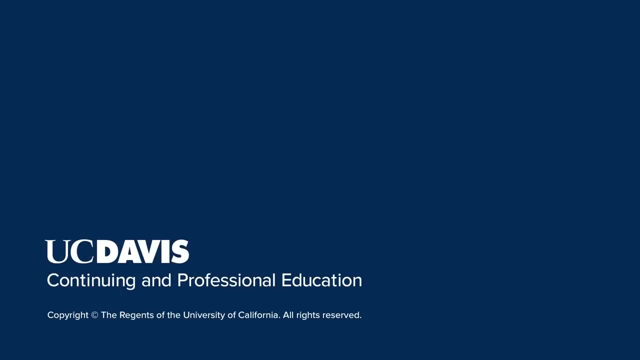 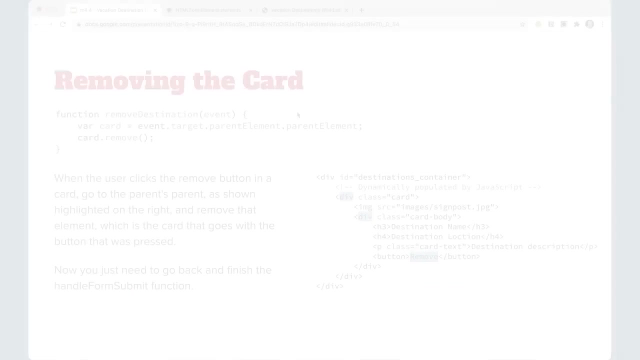 And a button, And then that gets added on there And then it gets returned. Great, We've got all of that in place. Let's save this And I'm going to pick it up in the next. The next step in this process is to actually write the function that removes the image. 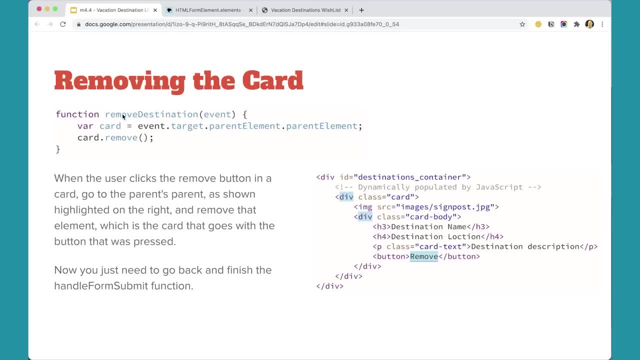 The function that removes the card. And that's what this is going to look like here. We're going to make a function called remove destination. We're going to pass in the event object so that when you click on that button, the remove button, that event gets passed through. 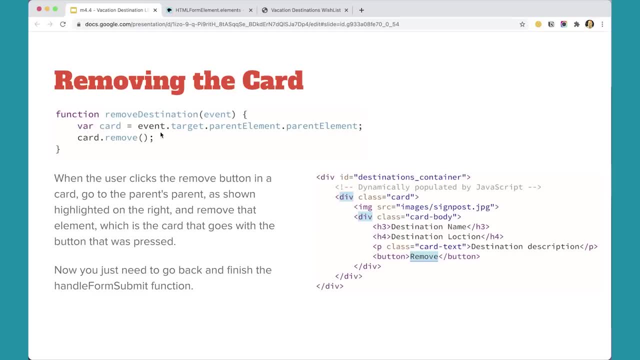 The event object gets passed through. I'm going to say variable card event, target parent element, dot parent element. So when you click this button I need to go up to this parent And then to this parent And say card remove. So I have to get up to that parent to actually remove that card. 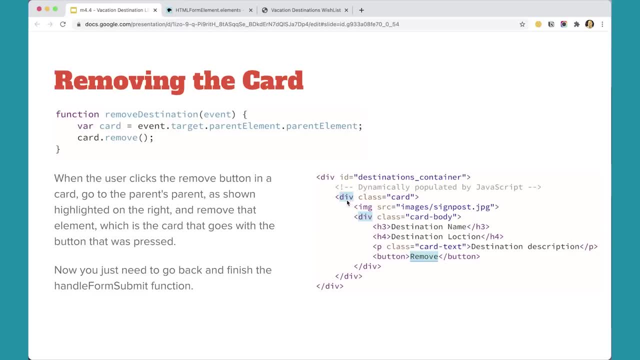 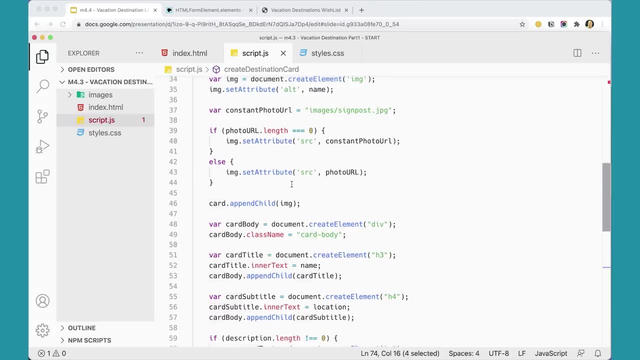 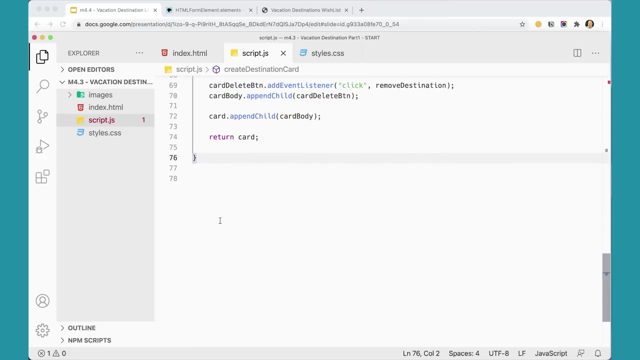 So I'm going up one parent to another parent to remove the card. So let's go ahead and add this function in over here. So down here I've got Function Remove Destination And it's going to take an event object. 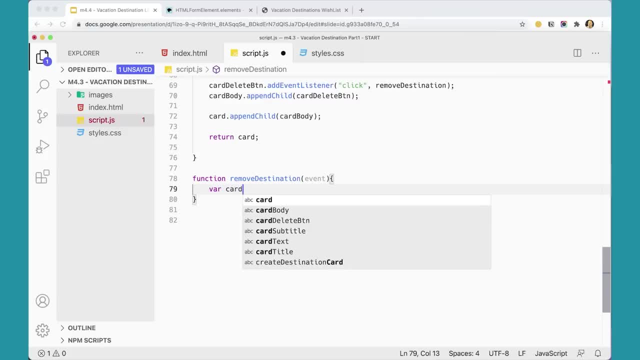 And I'm going to say: Bar card Equals Event. No, Yeah, Event, Yeah, that's right. Event. Target Dot: Parent, Parent element, Parent element, Dot, parent element. So that's going to be card. 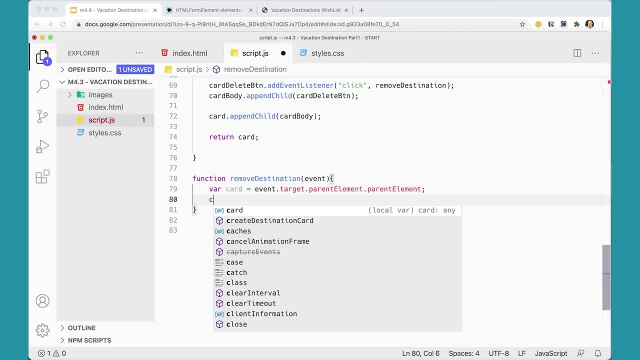 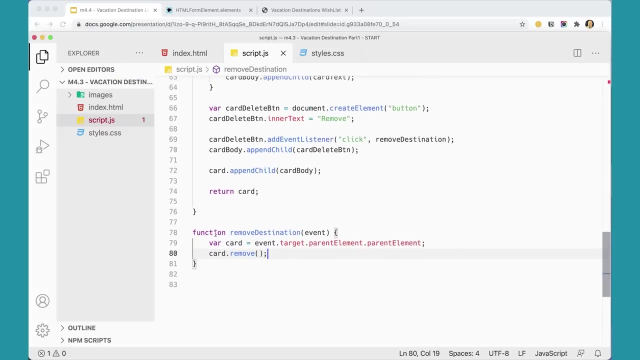 Once I get all of all the way up there, I can do Card dot Remove And that removes that card from The DOM. We hope. Okay, cool, So we've got our Remove destination Function. That's going to take in that event. 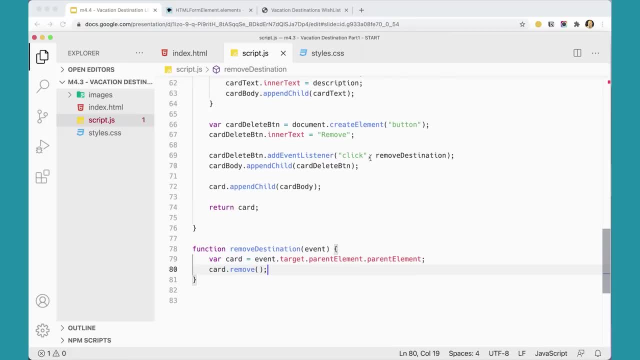 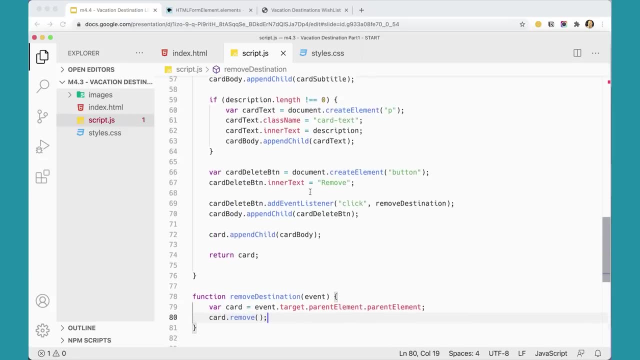 And then go up and actually remove that one, And that will get called here. If you get, If you click on The card delete button, Okay, cool, So we've got all of that in place. The last thing we need to do is kind of put it together. 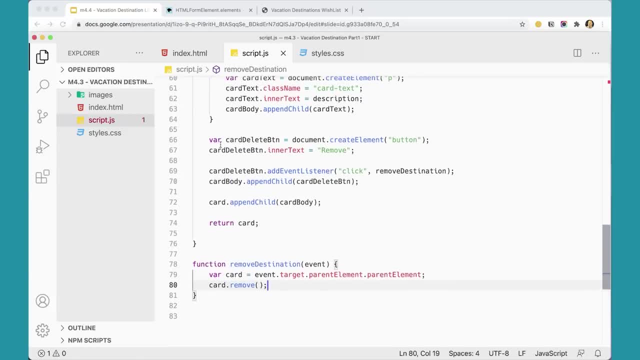 Up here, You'll remember, We had two things that we needed to do: We needed to create the card, And then down here, We needed to Actually add the card. So Let's do these two things And then we'll. 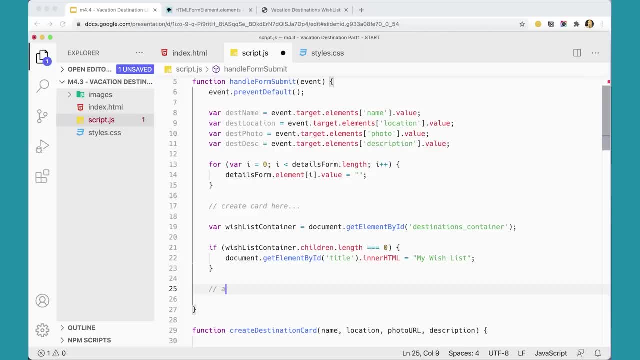 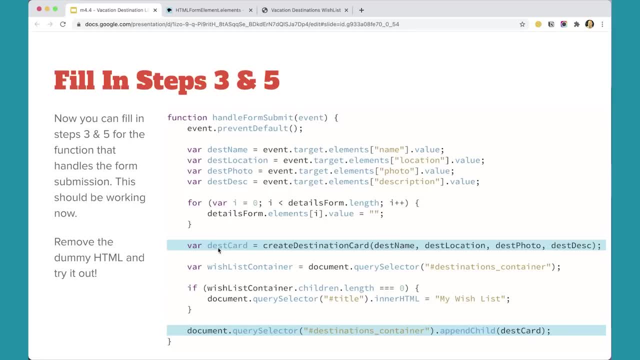 This is going to be the design. The~~~~ Then we're going to need Is Make a variable Destination card and that's going to run. That's going to be. This is going to be using A function expression here, So we're going to use a function expression to create the destination card. 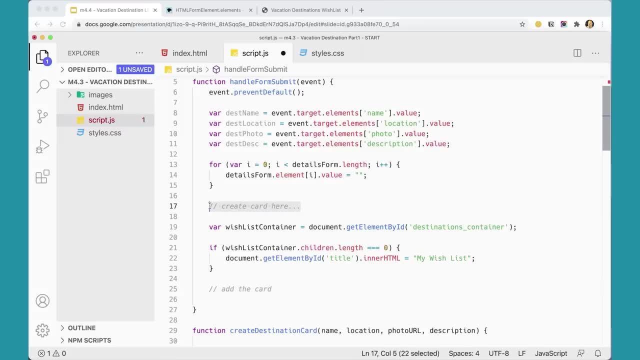 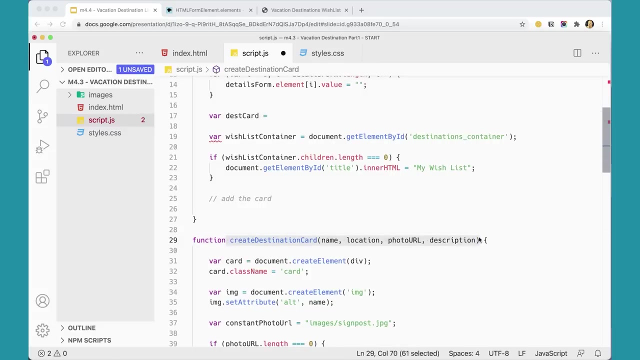 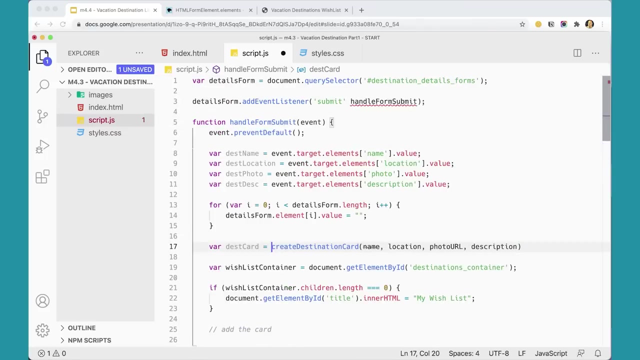 Passing in these variables. So let's do that, Okay. Okay, destination card. actually I'm going to short that, shorten it down to just dust card, dust card equals. and then what I'm actually doing is this thing here: create destination card, create the destination card. so I'm going to put that in here: create destination card. but what I'm 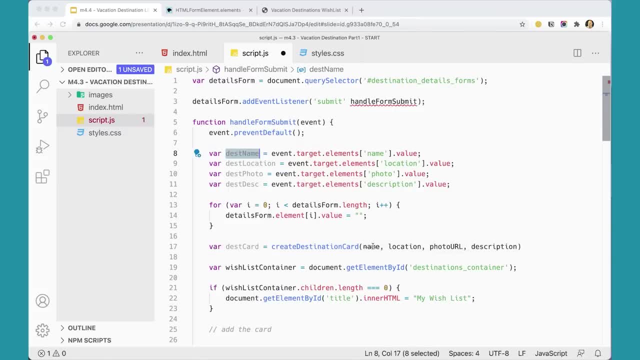 passing in is the destination name and I'm passing in the destination location and passing in the destination photo to the photo url, oops, and I'm passing in the destination description and then that should var. that's going to create. it's going to go in and create that. 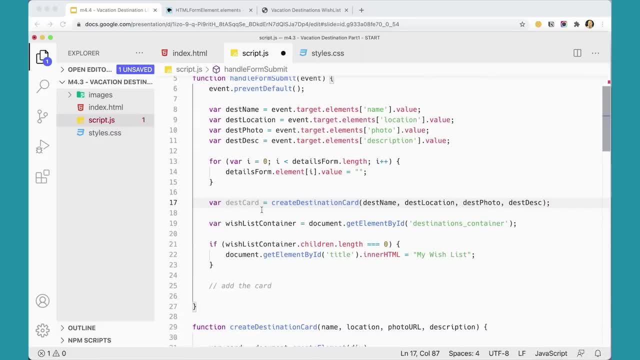 and then down here now I just need to add destination card, so that's going to say, okay, destination card's going to actually hold that card. and, remember, this function returns html, so that html for the card is now in dust card. because, remember, that's what this function does: create destination card down. 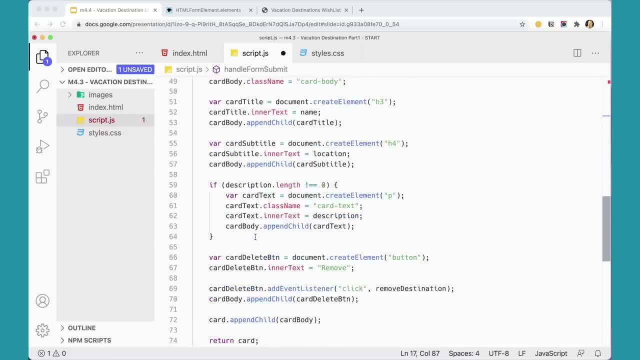 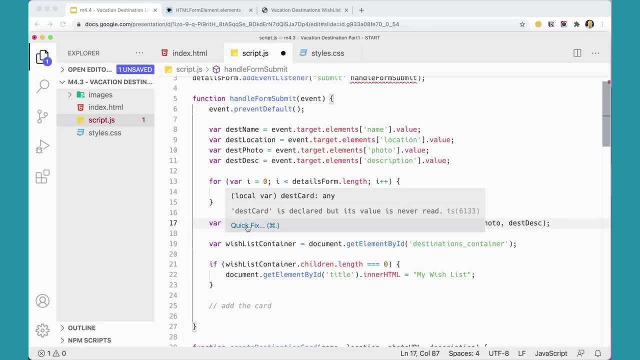 here. at the end it returns the card, which is the html for all the stuff in the card. so now, all of that stuff, all that html we created, is now in this little variable right here. it's in this bucket. okay, so the last thing we need to do: 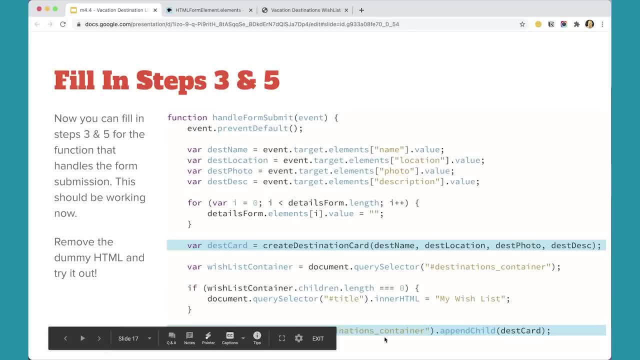 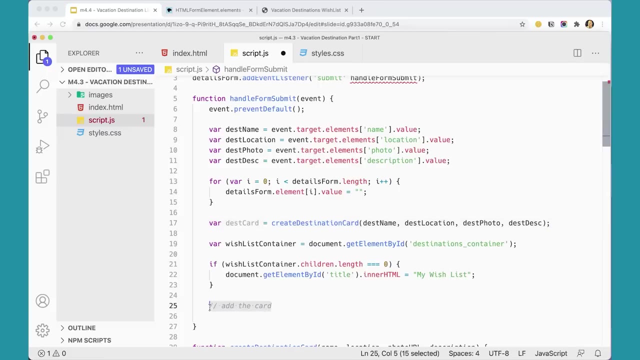 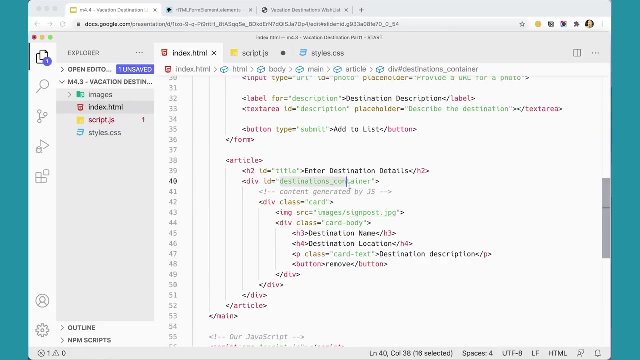 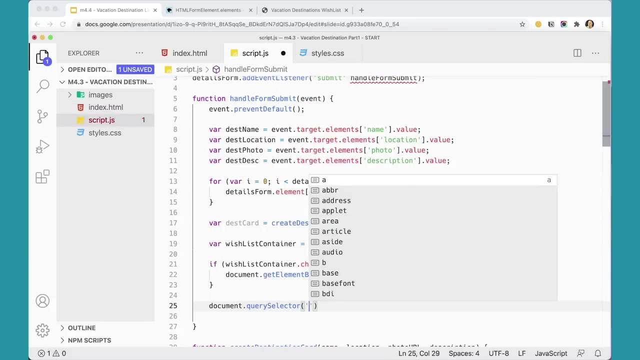 is: go in and find our container and append the child, right, so let's go ahead and do that. document. dot- query selecter. and what are we looking for? we're actually looking for this id here. quote: go get that id. dot- append child. and what are we adding? we're adding dust card. 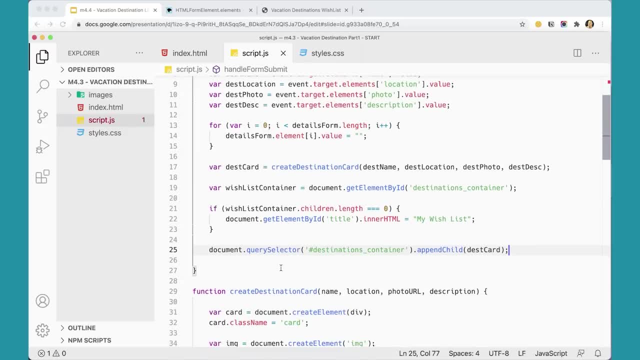 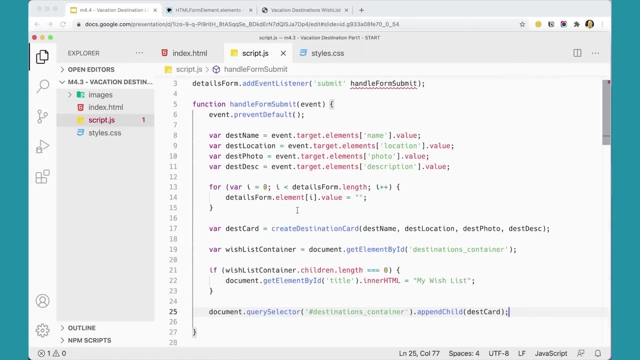 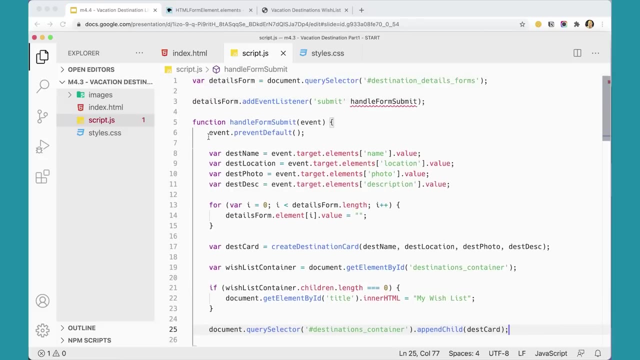 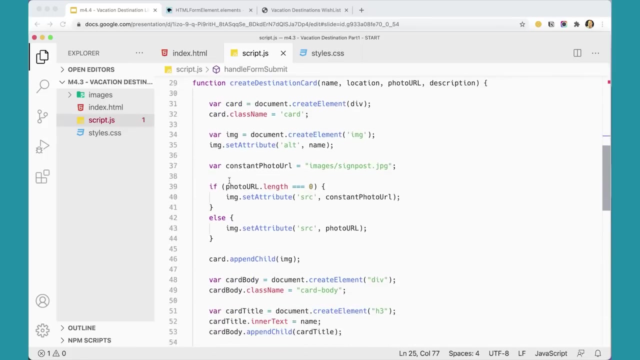 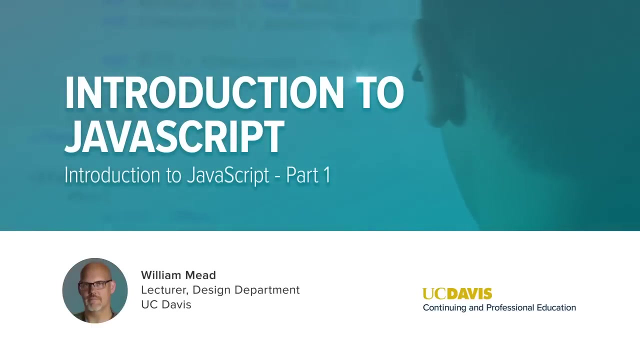 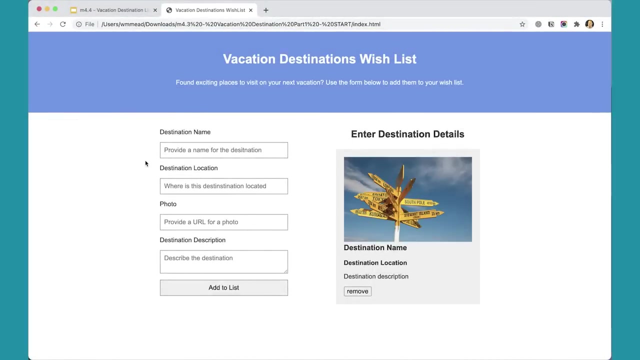 all right, cool, all right, great. now we've gotten all five pieces of our of our script together and in the next video we'll do some error checking and fixing of stuff and see if it all works okay. so all along as i've been working on that script, i knew that there was an error on it. 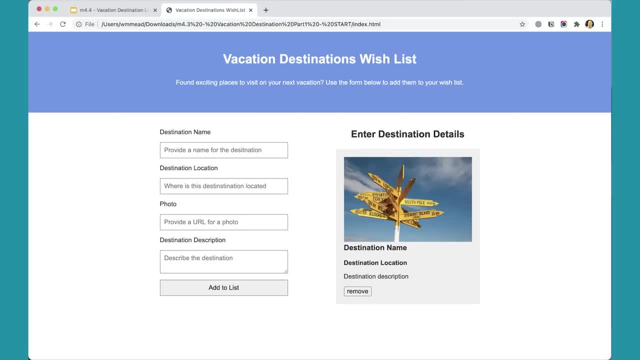 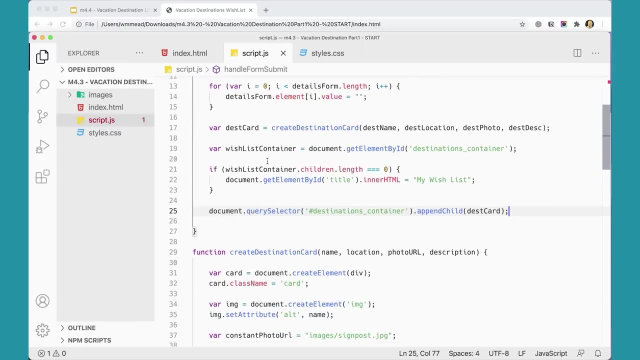 somewhere, but i didn't have a chance yet to test it, and usually you want to test scripts a little bit sooner than that, but i could tell that there was an error here because of this one and um, let's see what it is, and often you're going to have errors in your scripts and that's. 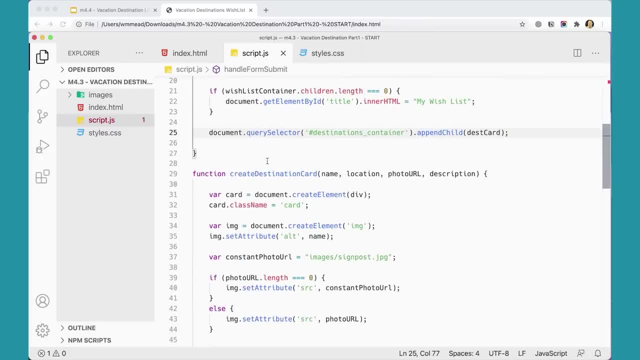 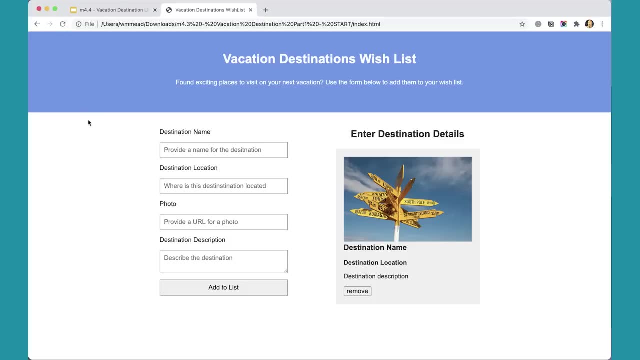 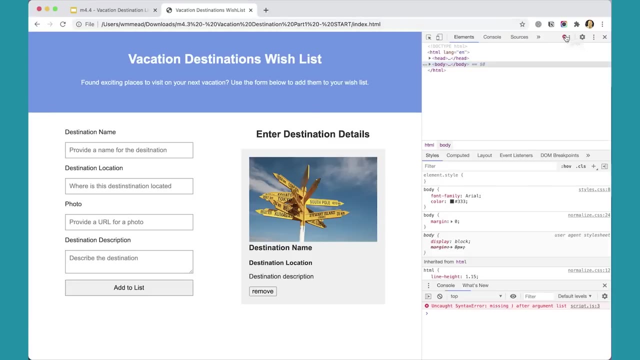 completely normal and, uh, you want to, you want to be able to find them. so i'm glad that that's in there and we can come over here. and if i just refresh this page and then run the inspector, you can see up here there's an error, error one, and if i look down here it says on line three: 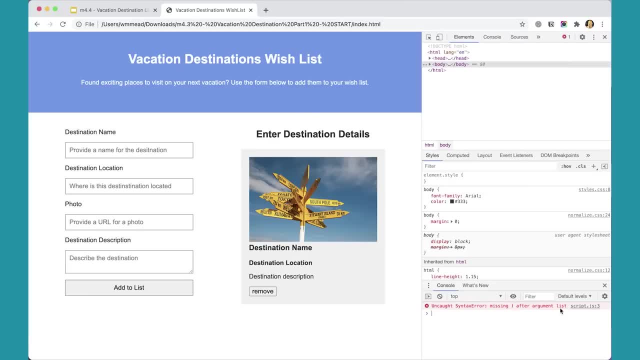 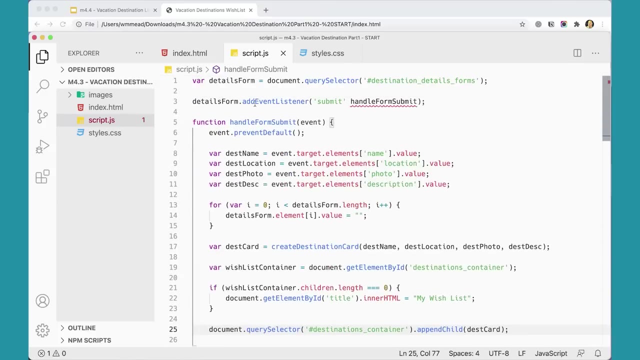 missing parenthesis after argument list. so let's go take a look at that and see if we can determine what's really wrong there, because sometimes those- um, those error messages are a little bit cryptic. so if i come in here and go to line three, i've got my ad event listener and i don't think i'm 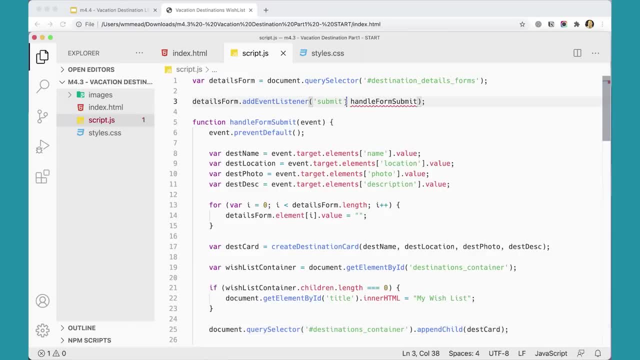 missing a parenthesis here, but i do notice that i should have a comma here and i think that that will fix this whole thing. and you know, a lot of times scripts won't work and you, you know you may feel like, oh my goodness, i'm completely in the, in a quagmire of misery here, but you could be. 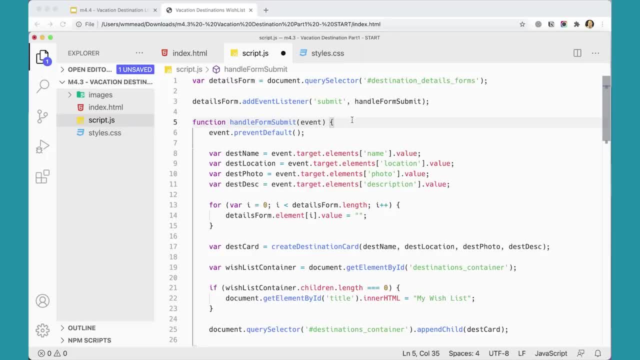 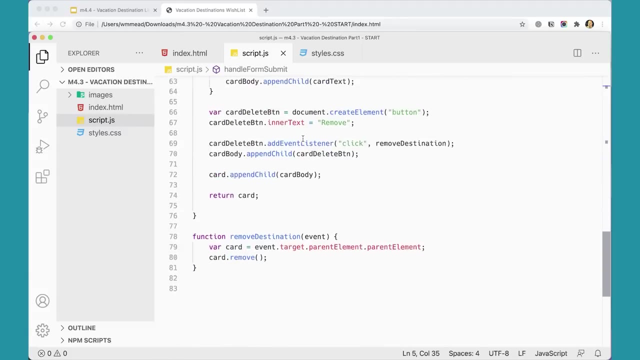 really close because i think if i put in that one comma it will work. if i'm off by one comma, that's pretty normal and can be kind of frustrating sometimes, but that's kind of the way life is when you're working with javascript or code in general. 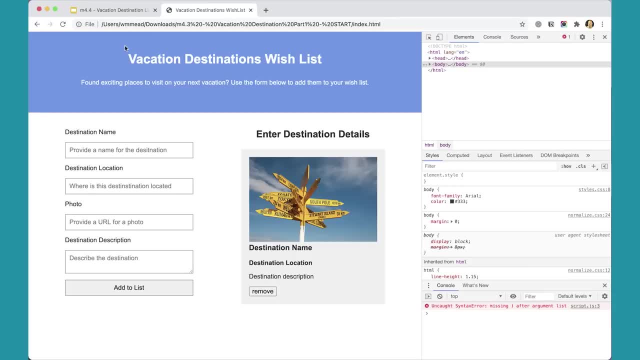 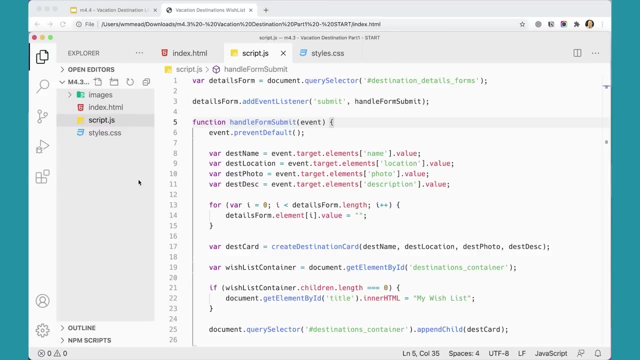 but let's see now if it actually works. if i come over here and refresh this thing and i still have an error, cannot read property of null on line three, do, do, do, do. let's see what happens. what else do i have here? on line three: handle form submit. 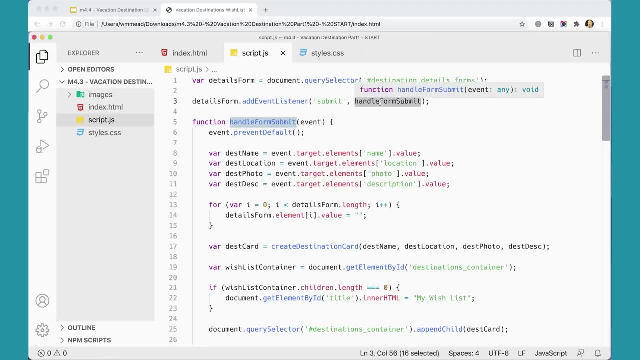 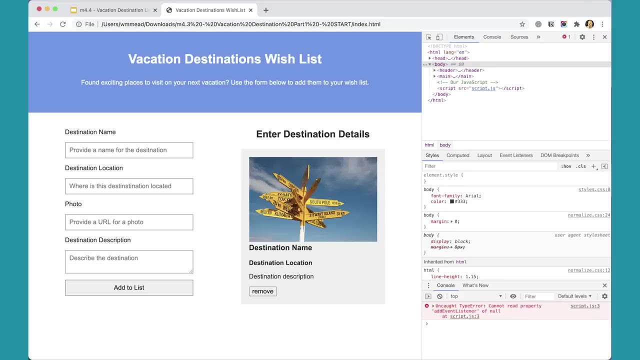 okay. so what i'm getting here is: this cannot read property of null, and usually that means something is misnamed somewhere. so if i come back here and look at this, i think the problem is that i'm not sure if i'm going to be able to read property of null or not. 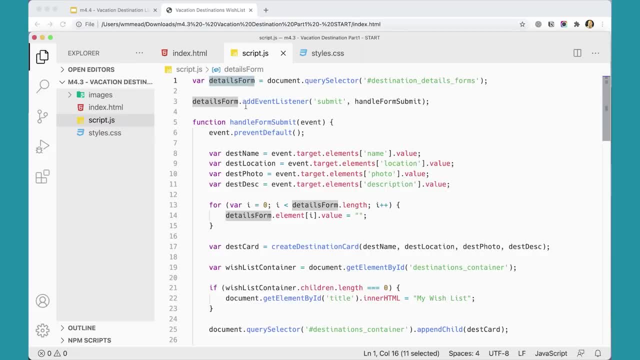 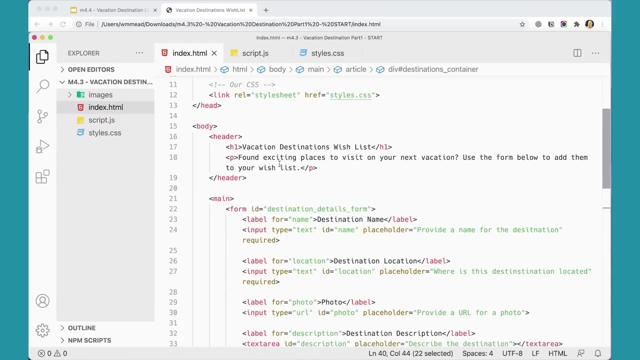 here is that it's saying i can't put an event handler on nothing. that's what the null means there. so i think the problem is here. destination details, forms: i don't think there's supposed to be an s on the end of that. let's come over here and check that. if i have my form here, yeah it. 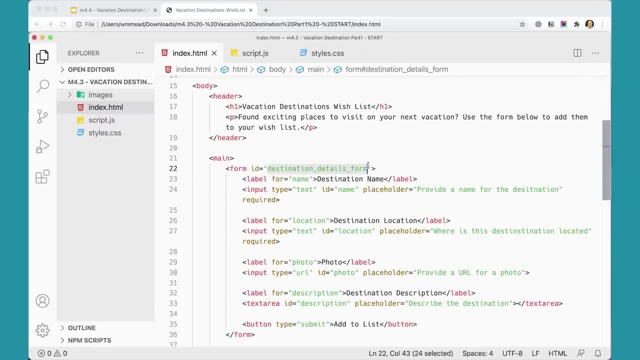 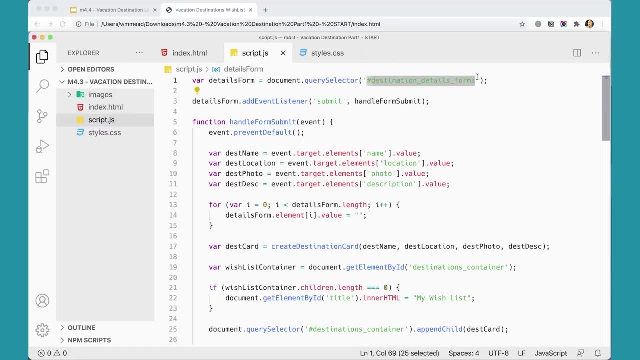 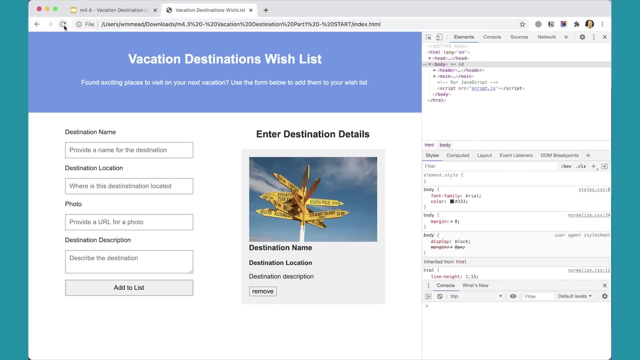 should be this id here. it's always best to just copy and paste these just to make sure they are exact, but it's really just the same thing about the s. let's give that a try. and now i don't have an error and i should be able to test this out, so i'm going to put a name. 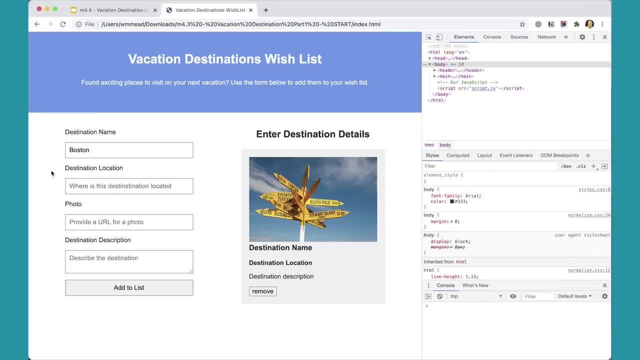 of a destination. let's try boston and it and uh, or let's try uh, annual hall. i think i'm spelling that wrong. we'll do Fenway Park destination location. we'll do Boston provide a photo. I've got a photo here per URL and I can put in a description here. 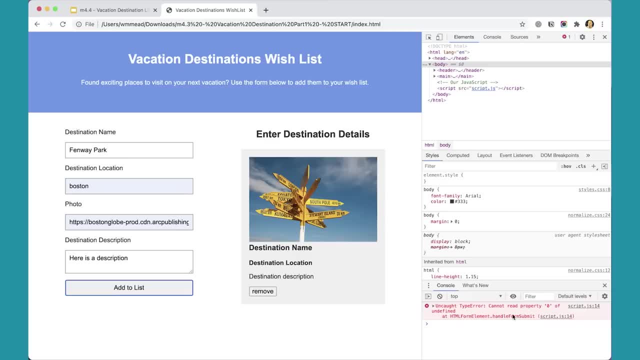 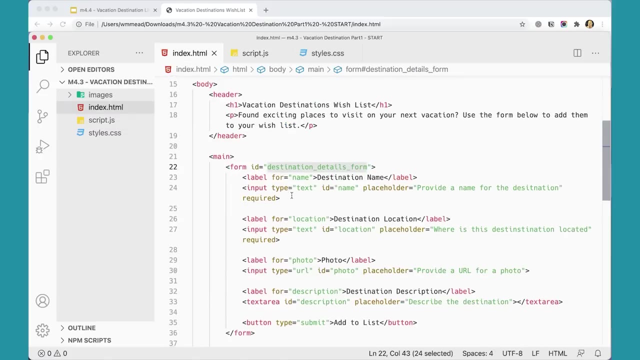 and click add to the list. and now I've got a cannot read property of 0 of undefined on line 14, so let's go back and see what's going on there. also, while I'm here, I should probably empty out down here. I should get rid of this card. I don't need. 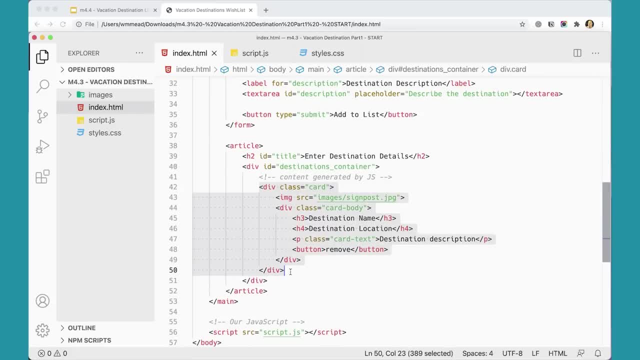 this one here anymore, so this one should come out all together. make sure you don't get rid of too much. they should line up here. this div closes down there, so make sure you're getting rid of just the div here like: so make sure this one. 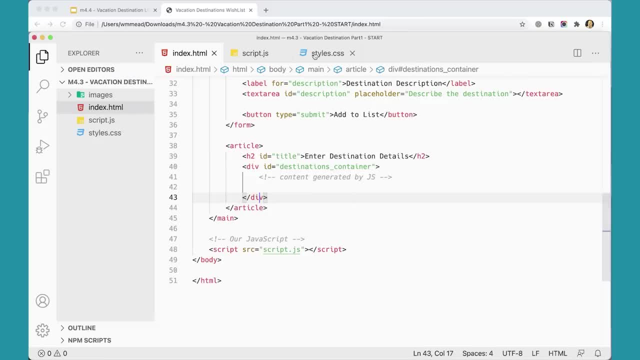 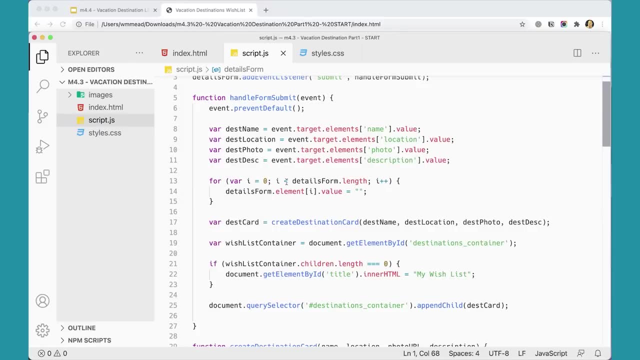 still closes, let's go over to script to line 14. so I've got a problem here. details: form dot length. it's got a problem doing the doing that script there. 2, 2, 2, i value equals 0. 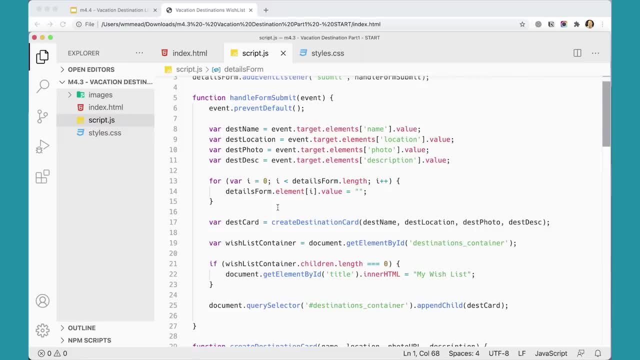 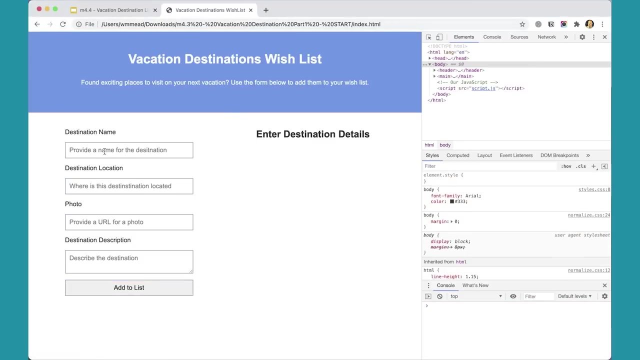 I see the problem here is actually: this needs to be elements again: an s off by one s. let's go back and test this. so now I've emptied that out, so that doesn't have anything in there at all. let's do this again. 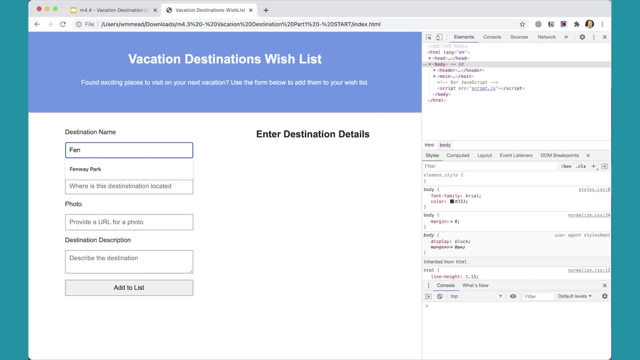 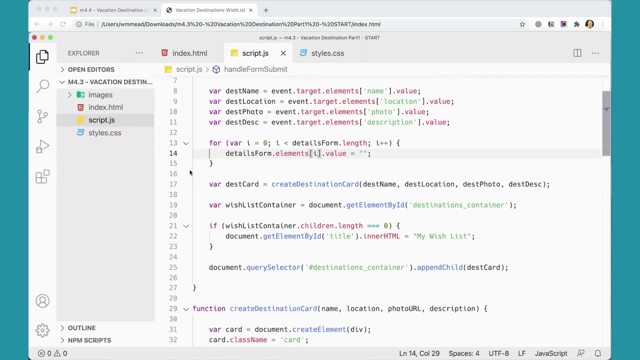 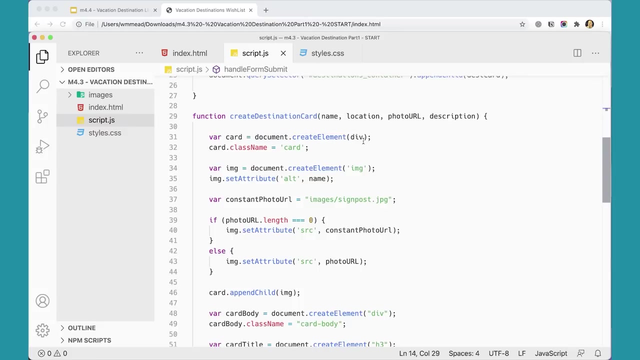 Fenway Park, Boston. I put my photo in there. here is a description. add to list. oh, reference div is not defined on line 31, so let's go back and take a look at it. line 31: line 31: var card document create element div. 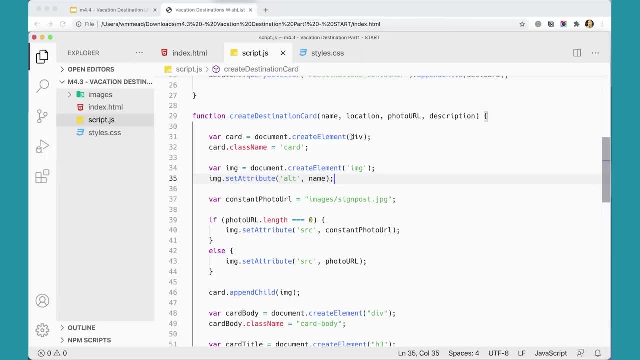 hopefully you can see. hopefully you can see right away what I did wrong here. it thinks that's a variable that needs to be in quotes. create element div: either single quotes or double quotes doesn't really matter. alright, good, so we're, slowly, we're working our way down the script. 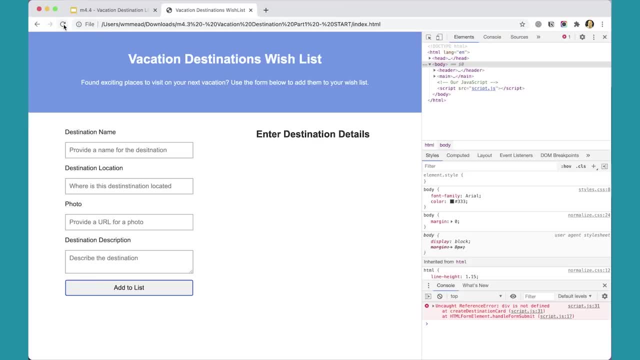 clearing out errors. it's kind of a long script to test. let's try it again now. let's do Fenway Park- I don't know how to spell that- Fenway Park in Boston- and maybe we'll get an actual thing here. add to list. add to list. 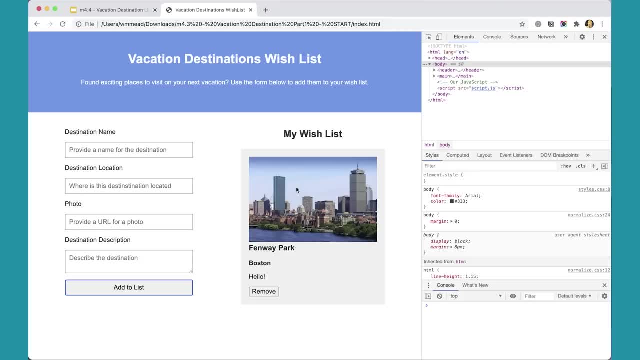 and look, there it is. we were able to add a card to the list. now we can check and see: does the remove card function work? it sure does. so we can now add cards and remove them from the list. let's try it again here. let's do. 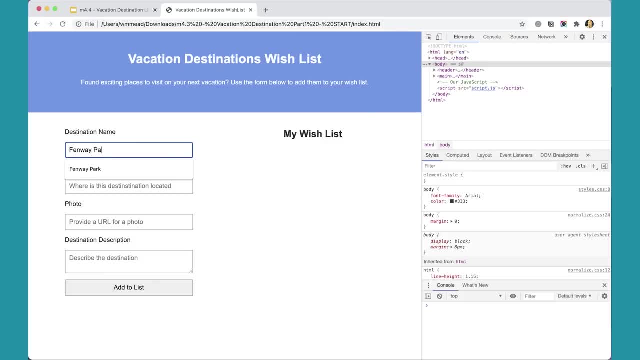 we'll do Fenway Park again and we'll do Boston, put in the photo that I have sort of in my form already. and then what happens if we leave the photo out? let's do that. no photo in there. see if the regular photo shows up. 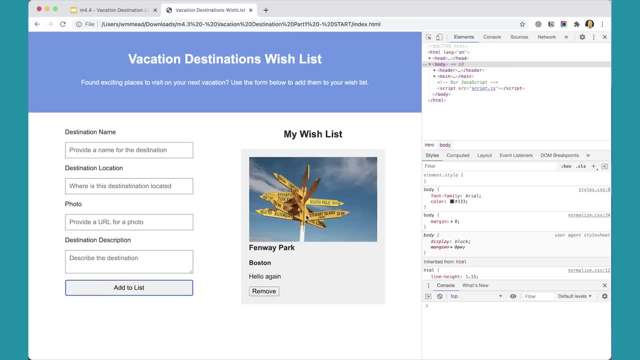 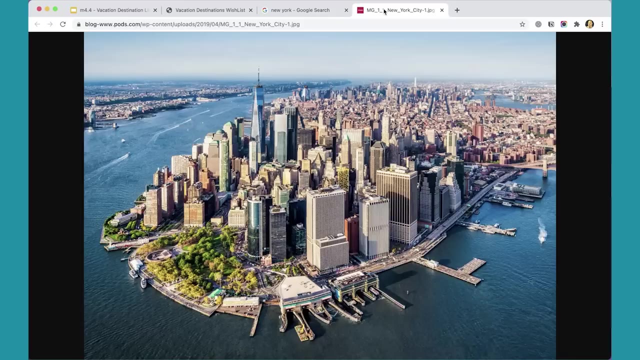 and it does so. that's the default photo and that's working. let's add another one. so over here, I did a quick search for New York and I found this photo right clicked and opened that photo up into a new tab, so here's a photo that I can use. 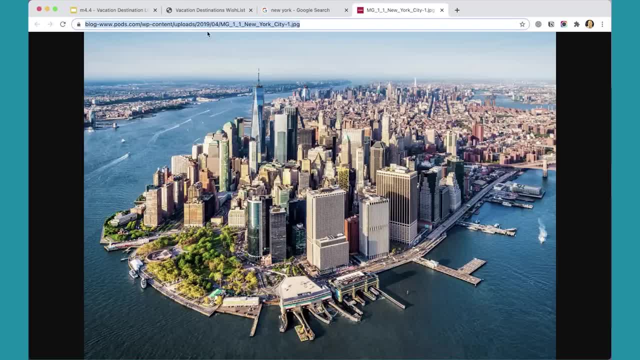 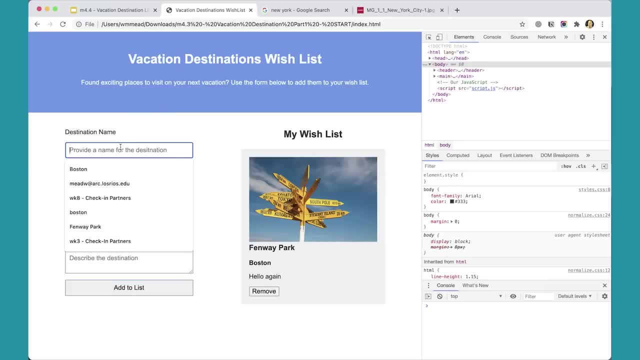 I'm just going to copy that URL and come back here and let's just do: let's say destination name: Empire State Building in New York, and I'm going to paste that URL in for that JPEG and then add a description: visiting New York. there we go. 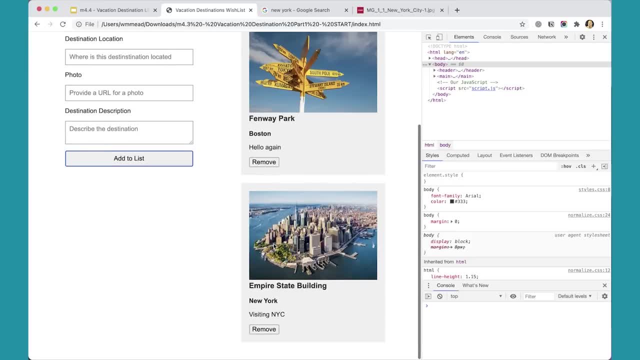 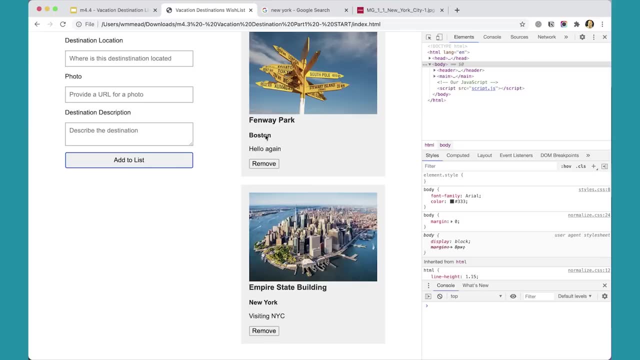 add to list and you can see that it's appended that card. it's added it to the list. so now I've got two here and they're both working. I can remove either one. if I remove this one, that one will go away and the New York one will stay. 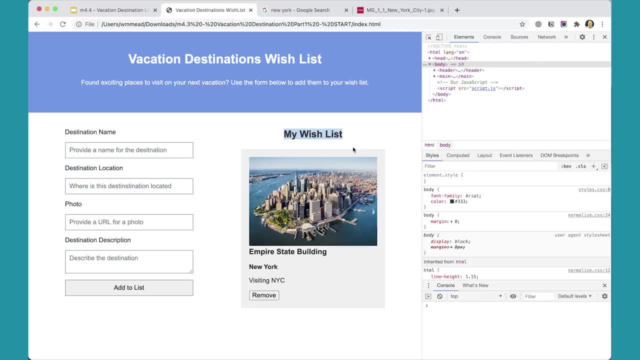 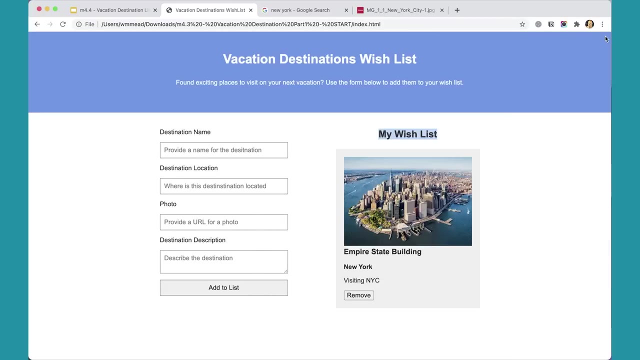 notice that the header here changed as it was supposed to change, so everything else is working. so here in this little application we've created here- and it's not very sophisticated, it's only got a few features, but we can add elements and remove elements on the page. 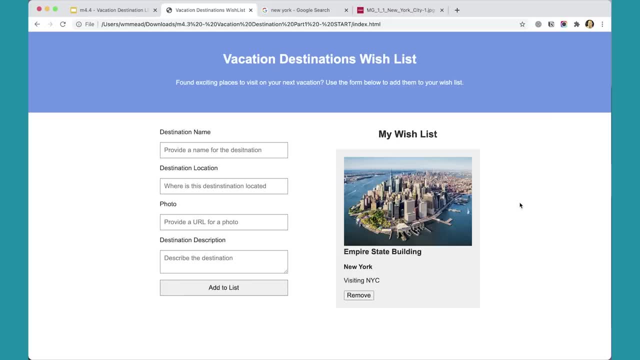 pretty easily with a little bit, with a little bit of scripting effort there, and this is a really great sort of capstone project for the end of the course here. now our last final pieces here are to refactor the script down a little bit and use our best practices. 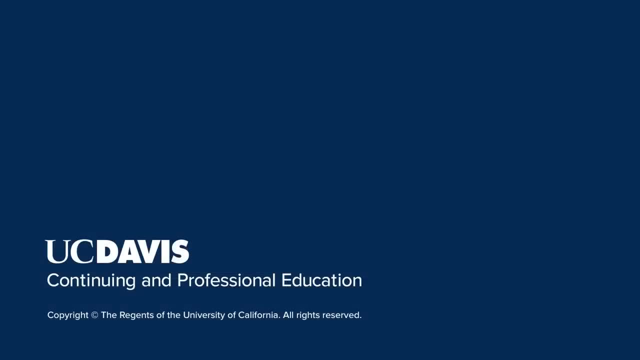 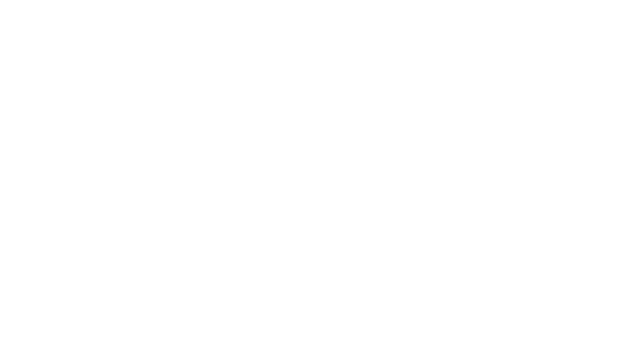 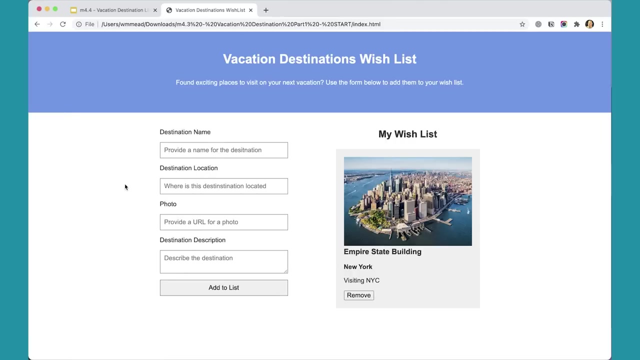 and we'll do that in the next video. okay, now that we have a working project, which is great, and we had some errors, and that's normal, and I'm glad they appeared here for me because they'll certainly appear for you- it's very easy to end up with. 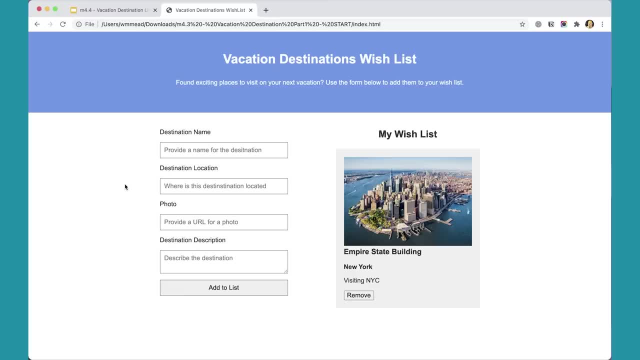 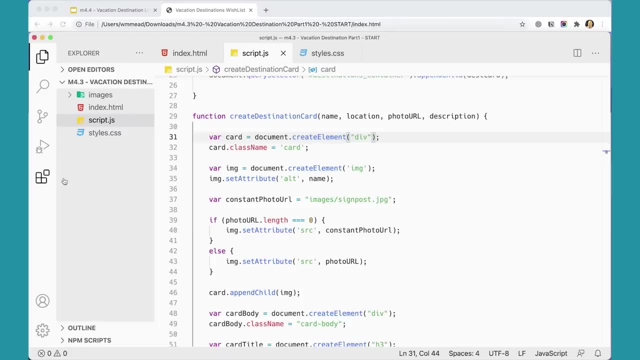 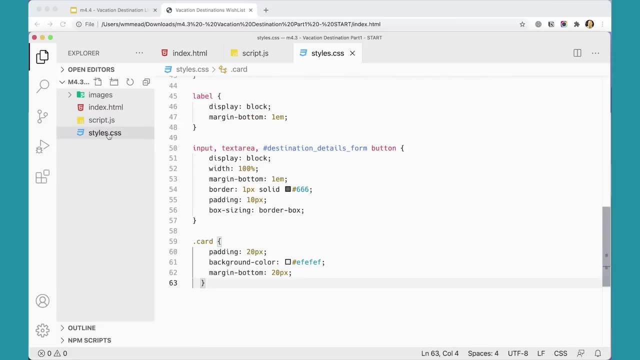 little mistakes, whether you spelled something wrong or used the wrong ID. there's a lot of moving parts with a little web application, even one small like this. you have your HTML with IDs that things are hooking into. you have the styles where there's, you know, different elements that are affecting 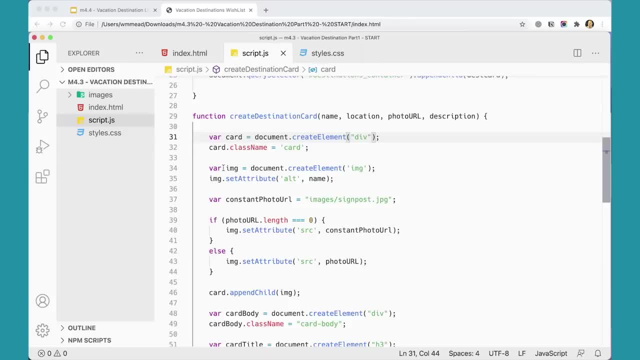 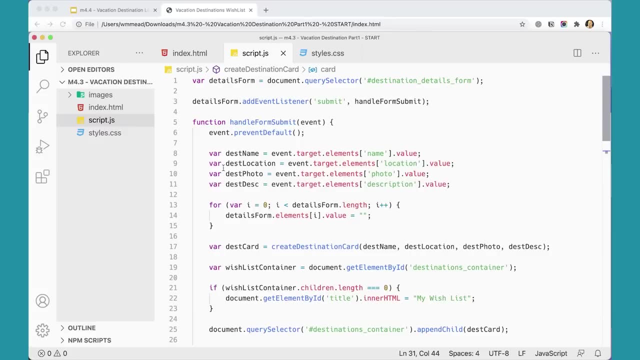 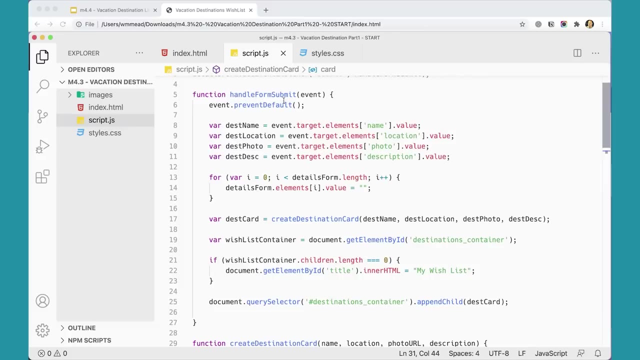 the way the page looks and then in the script you're sort of manipulating many times both of those things kind of on the fly. and just for a quick summary of the script here, where when you submit that form what we're doing is we're running this handle form, submit function. 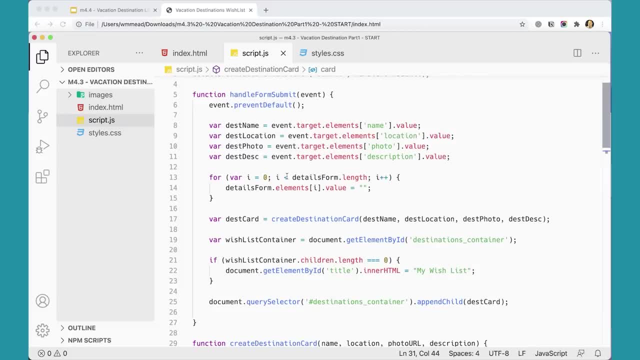 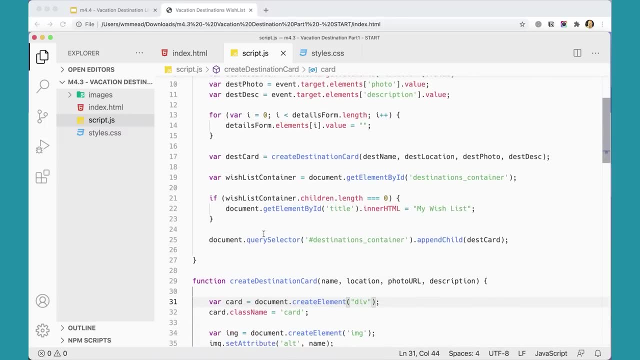 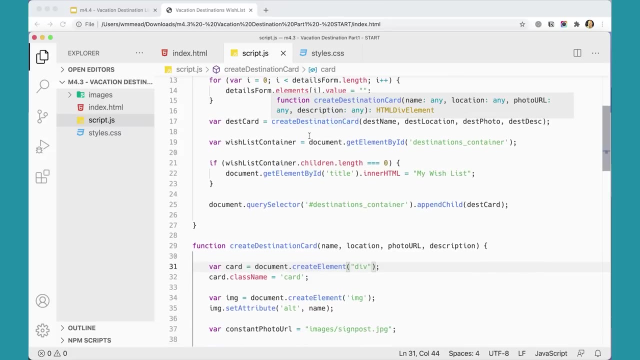 which is getting the values out of the form, clearing out those values from the form when it's done and then going through and actually creating the actual card and then after that, going in and fixing the header at the top of that container at this part of the page up here. 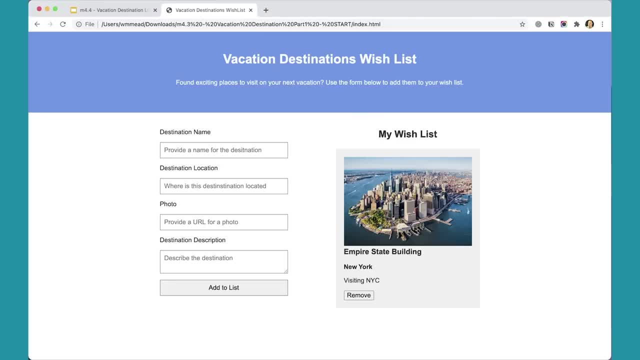 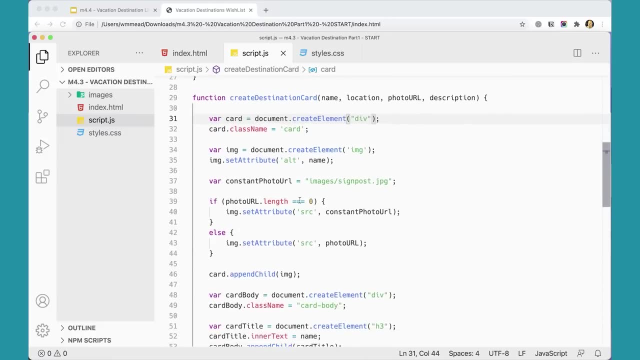 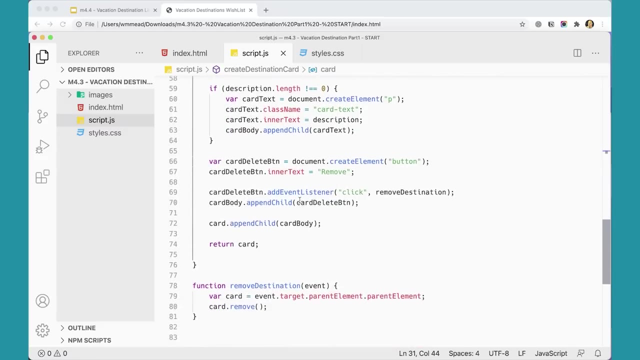 over here fixing the header if we need to, and then after that we actually put the card on the page. and the create destination card is a long function because we're creating each one of these HTML elements manually or individually here, having JavaScript create those elements and put the contents inside of them. 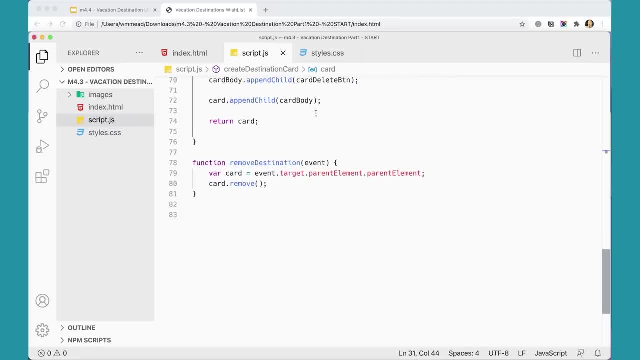 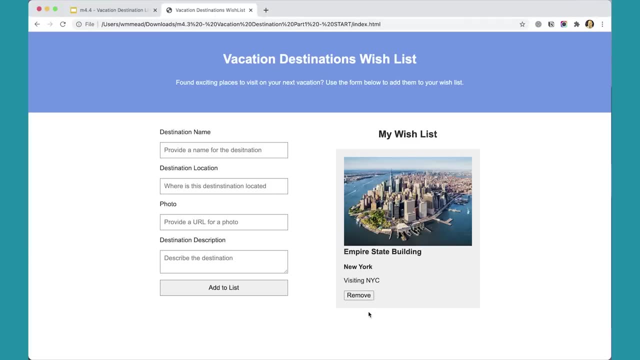 and then add them actually to the DOM as they're needed. plus, we have an extra function that allows you to remove a card. so that's one more extra piece of functionality that we have in this little application. the last thing to do is to kind of clean it up. 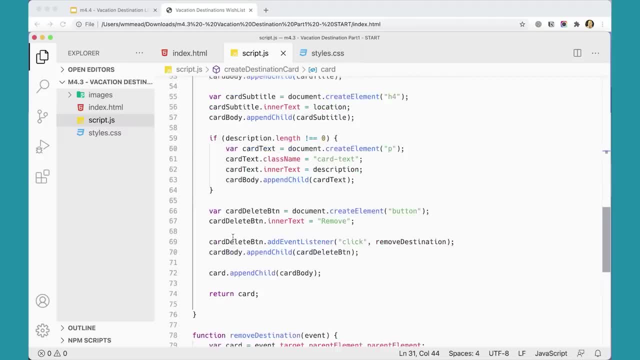 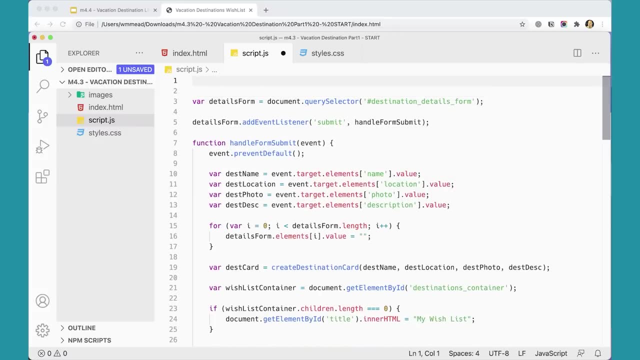 with our, by adding our function up at the top here to enclose the whole thing and then changing out the variables. so again, we would just do open parentheses and run an anonymous function with its parentheses and its curly braces and then one more set of parentheses to make it run. 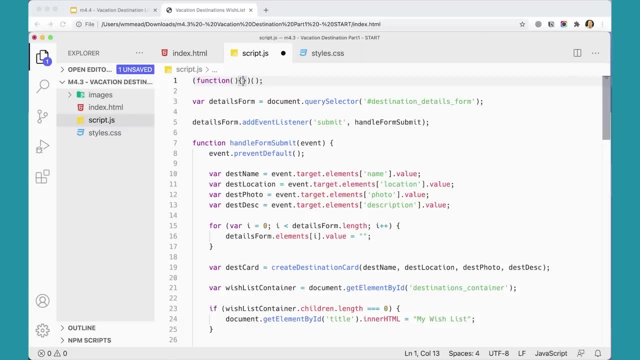 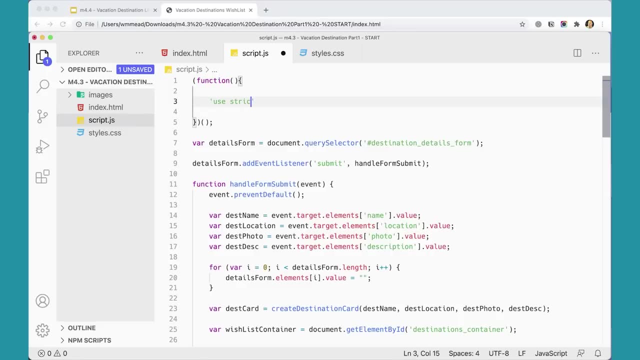 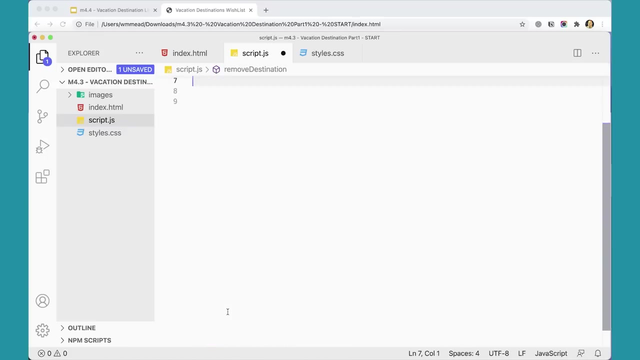 so this will run when the page loads, so I can move this down and I can stick in here, use strict and that will make sure that I'm not introducing any variables by accident in the global scope, and then I can take everything that's in here and stick it inside this function here. 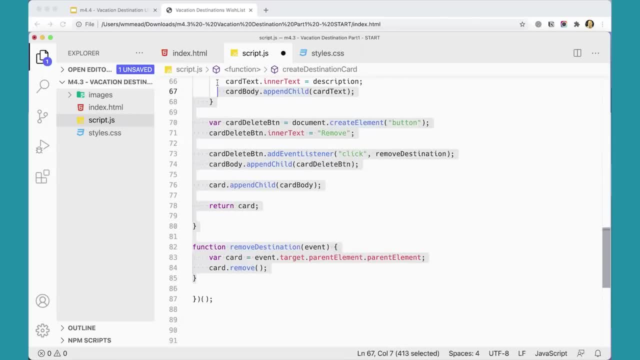 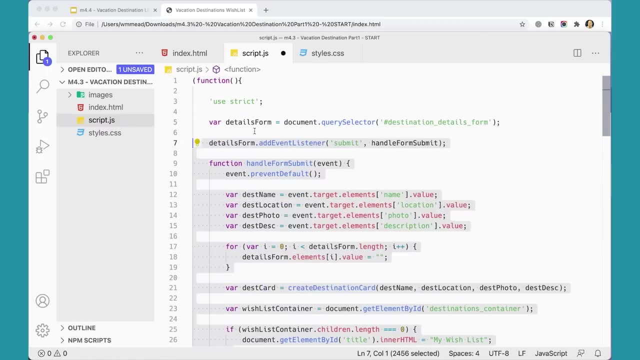 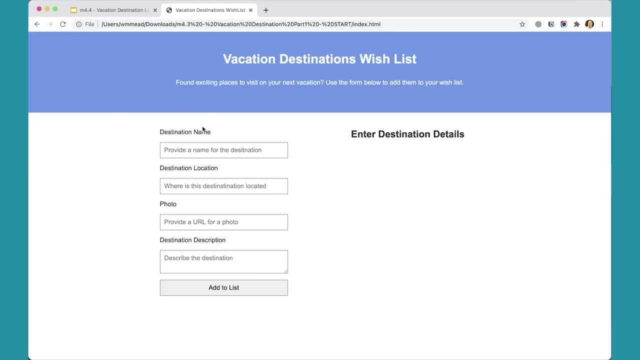 and I may need to tab it in once. there we go and that should look good. so that should still work the same as before. we can test it. what was I doing? Fenway Park- oops, I can't type Boston. so there's the Boston line and that still works. 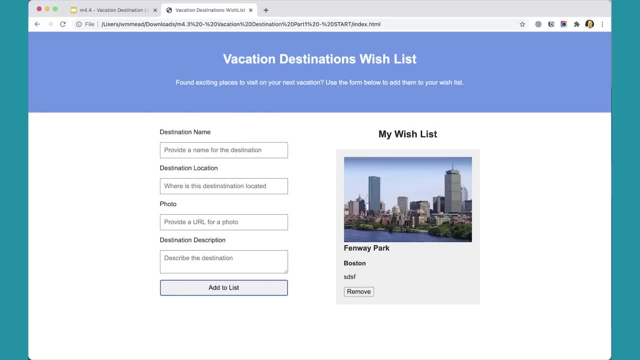 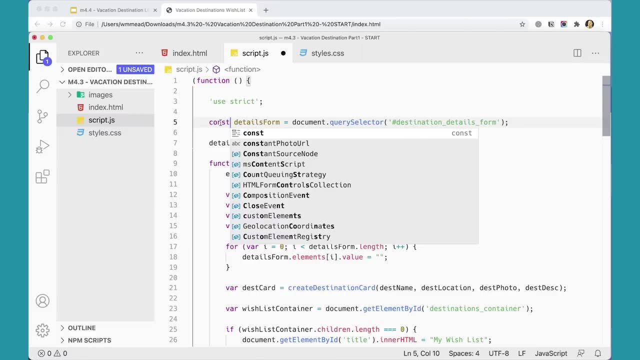 so that's great, so we've got that. and then the last thing you could do is go through and replace all the bars with const or let- and they should be const as much as possible, so we can just put const there. come down through here, that's going to be const. 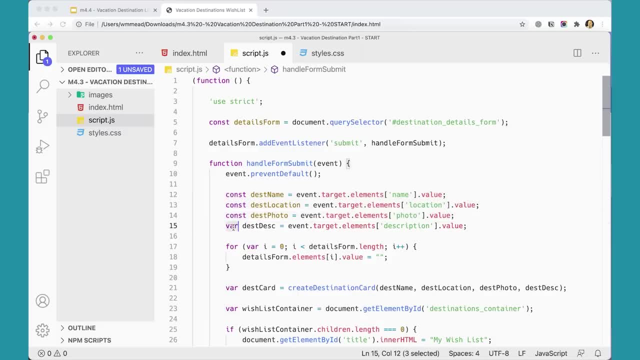 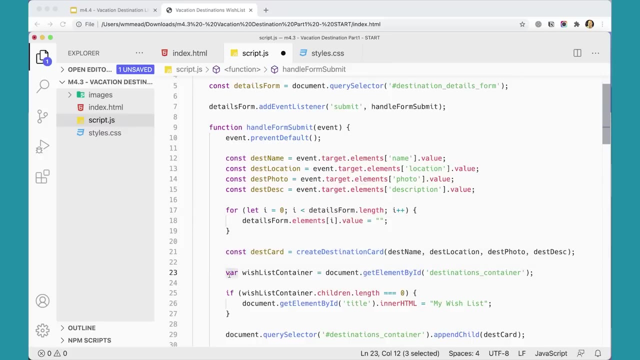 that's going to be const. all of these can be const. now, this one needs to be let because that's actually in a loop, so that's going to need to be let. and then, down here, this can be const. that's a container, so that's going to be const. 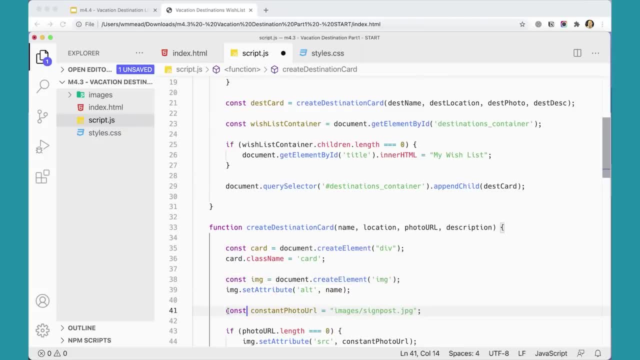 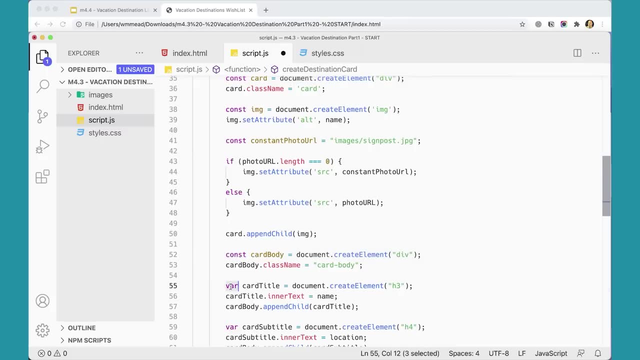 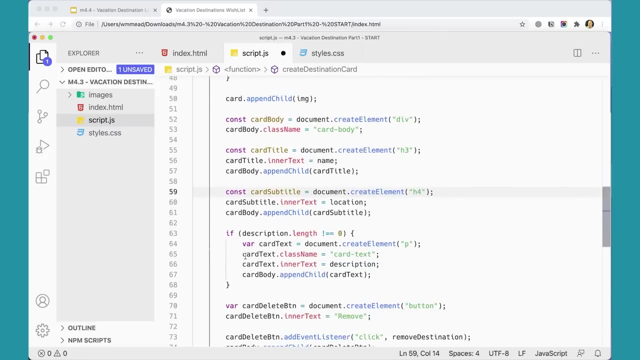 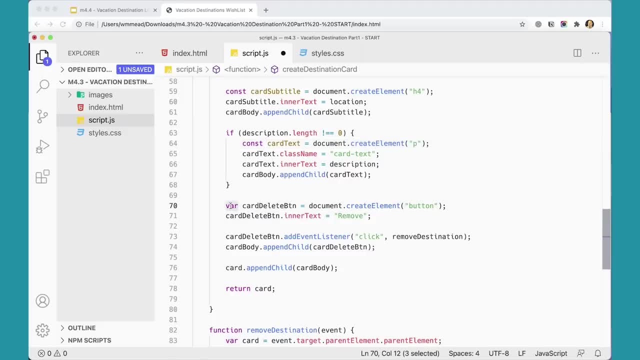 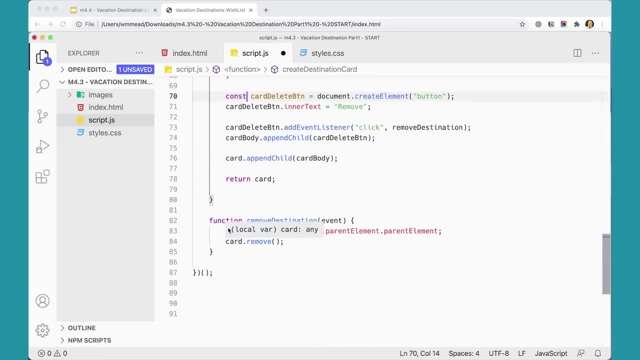 and that's certainly fine as well. I, just as you're new, when you're new at this, I think it's helpful to start with var and then come in and add const as you need to, or let, and again let is for if the value is going to change. 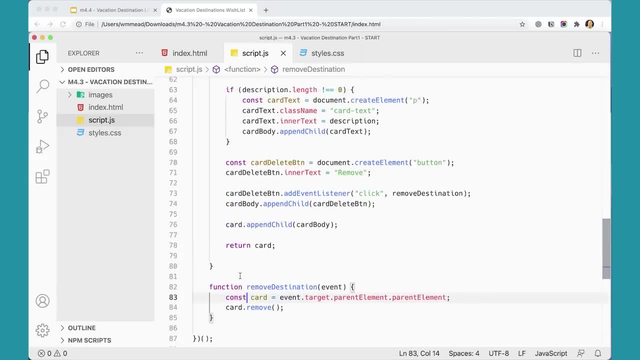 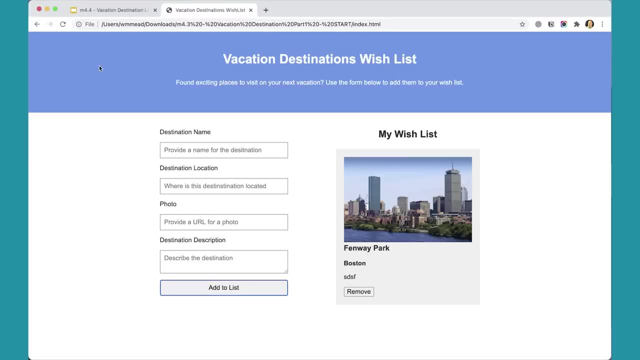 none of these other values are going to change when the script runs, just the one inside the loop. I think that's the only one. I could be wrong. let's just check and see if I am wrong. and if you are wrong you'll get an error and you can fix it. 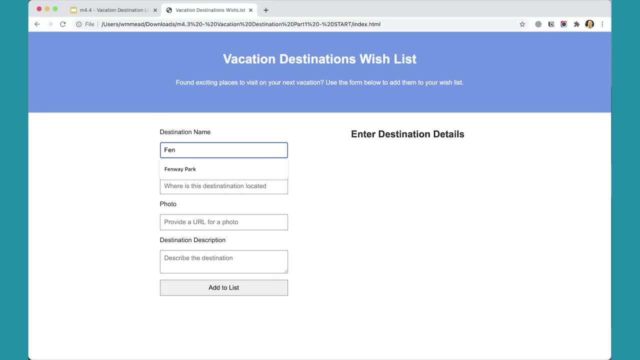 so if I refresh this type in Fenway Park one more time- Boston and the URL- and look at that, it works great, click remove and it removes it. so everything is working the way it should. this is a really great capstone project that sort of brings together 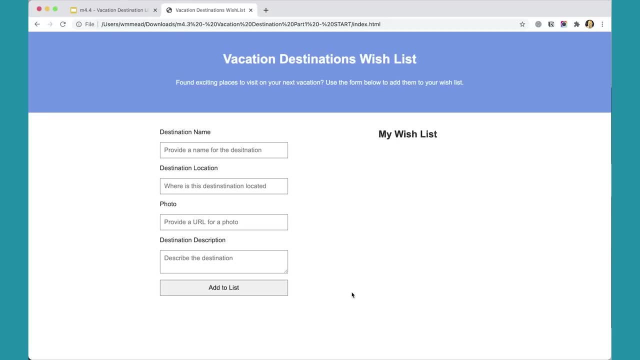 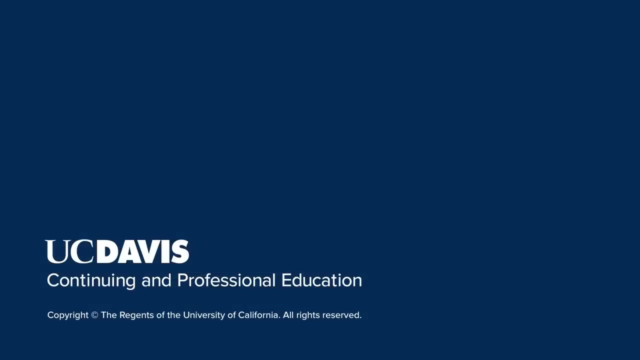 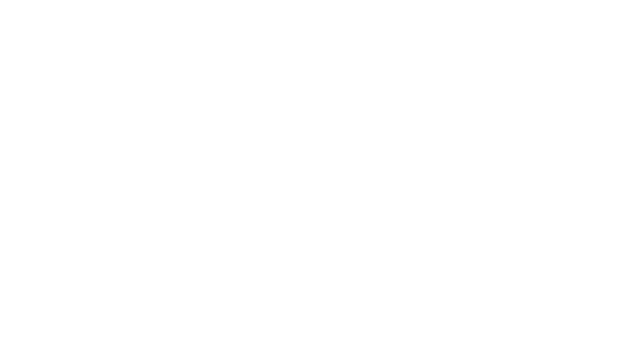 everything we've done in this first course of this specialization and I look forward to seeing you in the second course of the specialization, where we'll get into jQuery and creating all kinds of cool interactive elements on web pages and more. congratulations, you've made it to the end of our first course on. 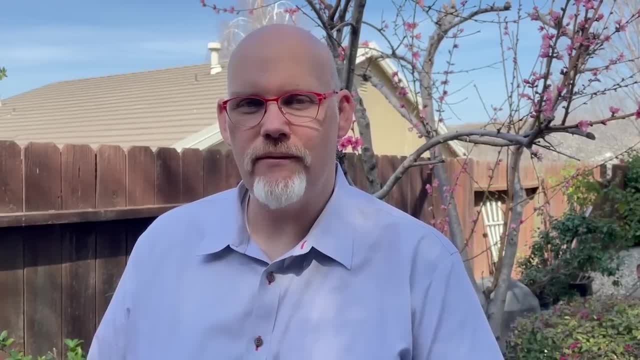 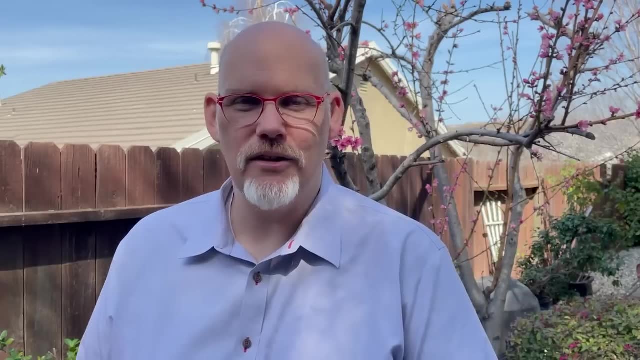 JavaScript. I hope you've had a lot of fun with it. I hope you've had fun doing it with me while I stand outside. outside here in California in this beautiful day- not that many miles away from where JavaScript was invented over 25 years ago. but JavaScript's a lot of fun. 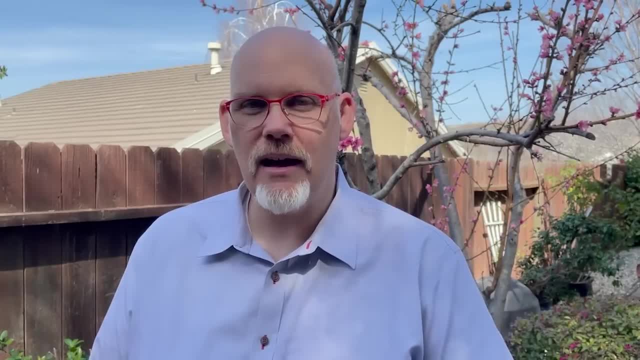 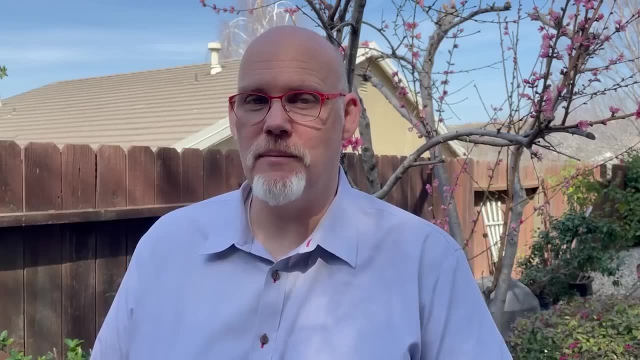 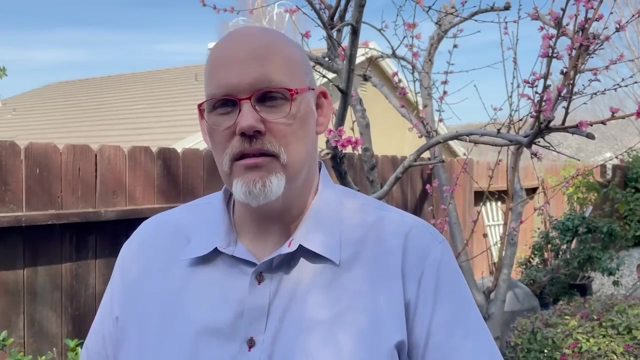 and you've learned a lot. so you should give yourself a pat on the back, and i hope you're excited about the projects we've done so far. also, i hope you realize that there's a lot more to learn about javascript and that you'll join us in the next course in the specialization, where we get into jquery and we look at some of 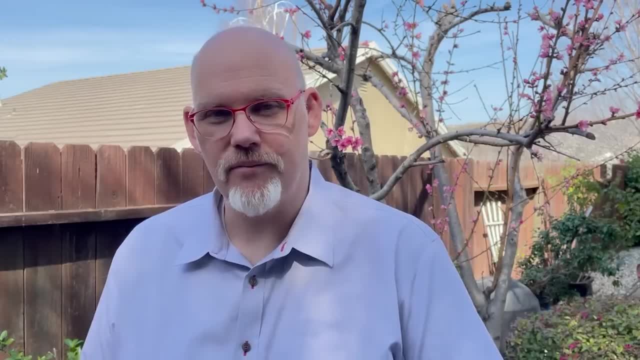 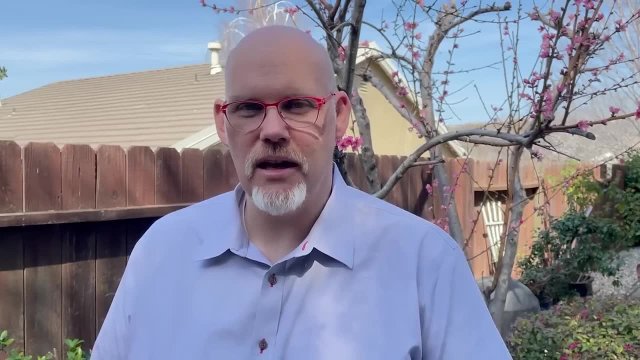 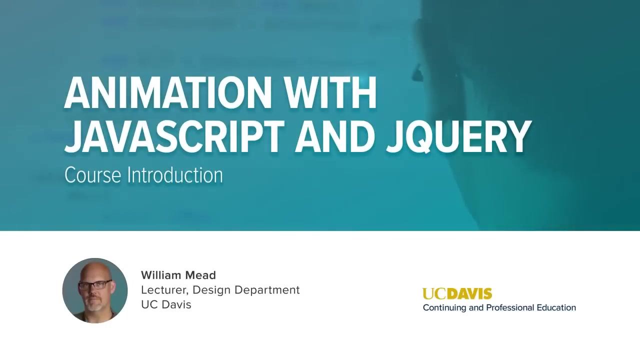 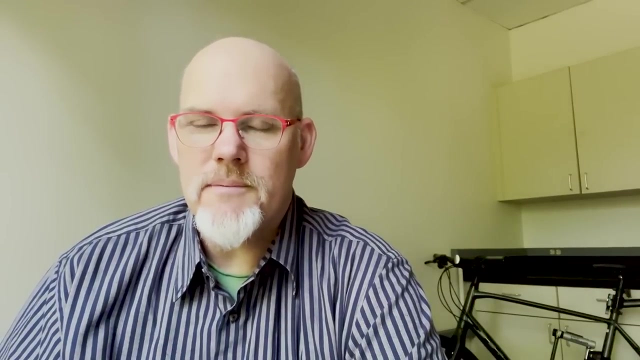 the cool things that we can do with the jquery library and some of the cool interactions that we can make. so thank you for coming along this far and i hope to see you in the next course. hello, my name is bill mead and i'm back again for our second course on javascript in our javascript. 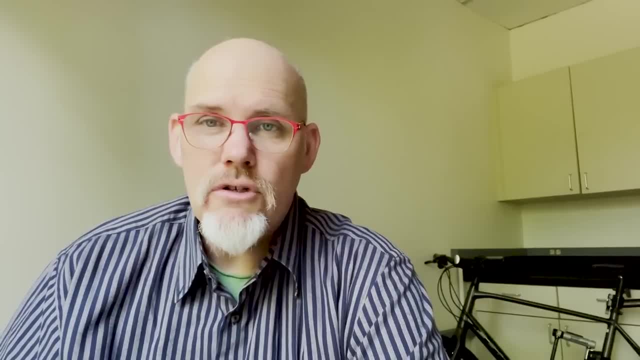 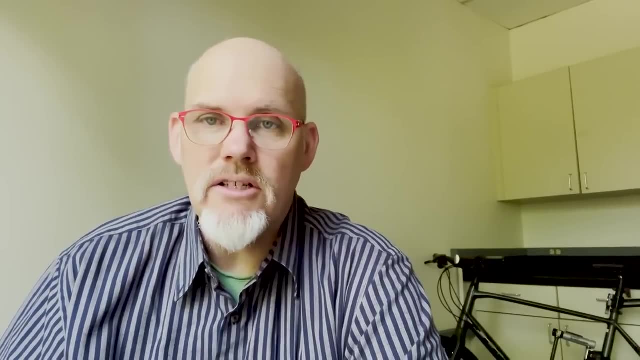 specialization. hopefully you finished the first course. in the first course we covered a lot of basics, uh, learned a lot about the syntax of javascript and got a lot of really great practice and built some fun projects. this course we're going to take it even further. we'll introduce the jquery library. 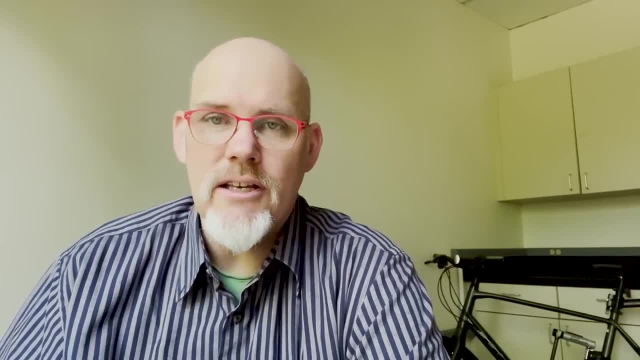 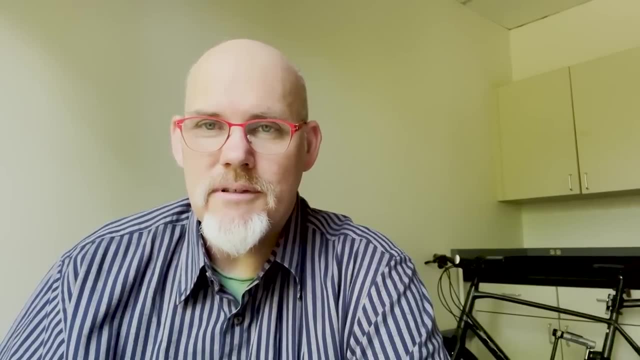 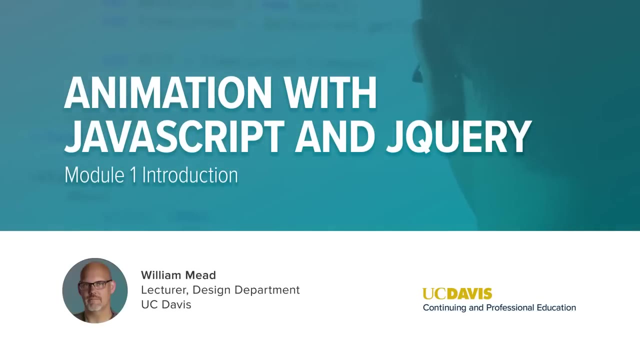 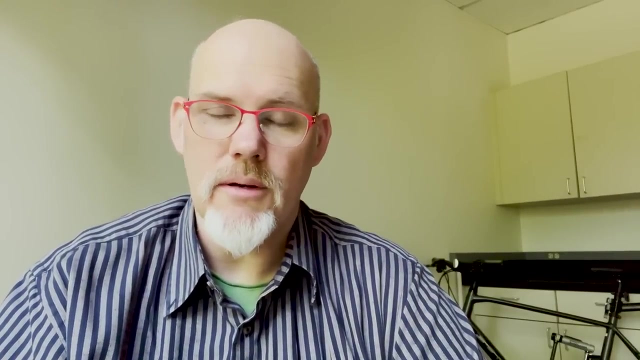 we'll build some more complex scripts and we'll really build up your skills in javascript. so break out your code editor and let's get started in the second course on javascript. hello and welcome to our first module in our second course on javascript, in our javascript specialization. 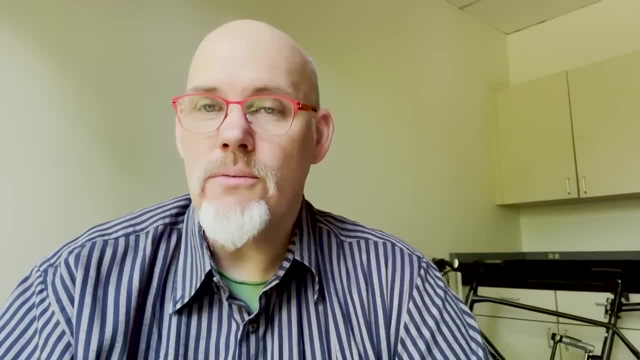 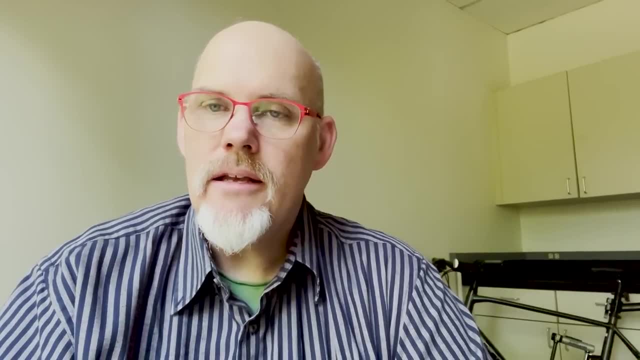 and in this module we'll really get into. we'll start working with the jquery library and learning about what that library is and how libraries can work with javascript, and then we'll compare jquery- the syntax of jquery, to the syntax of plain vanilla javascript and by working with 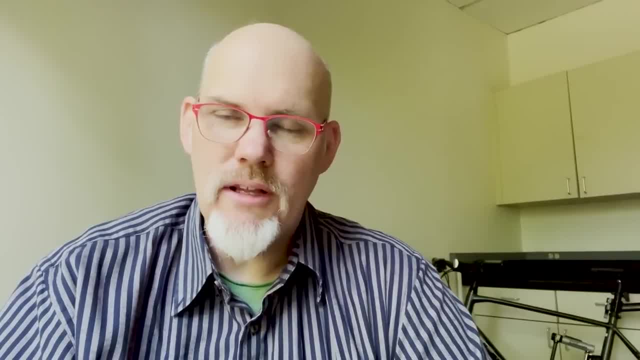 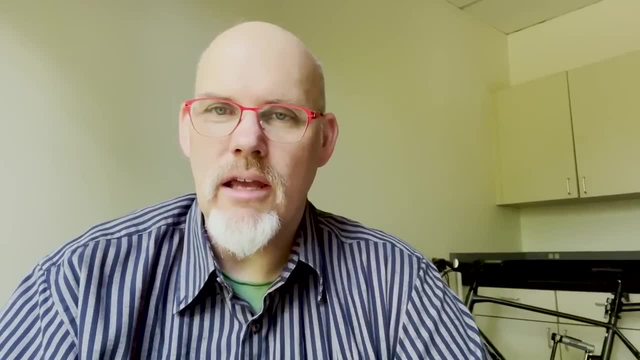 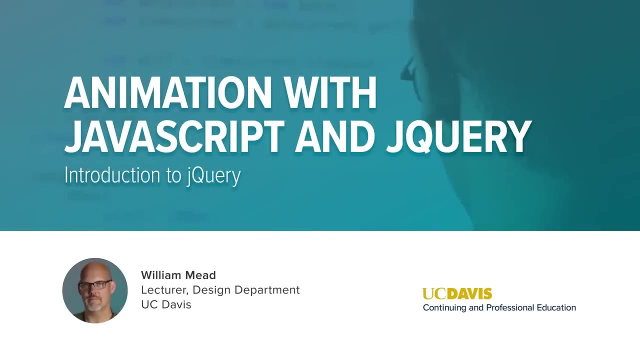 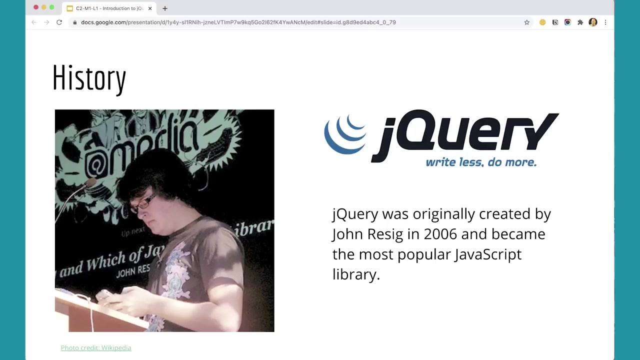 these two together. you'll learn a lot about both, and that's really helpful, and along the way, we'll work on some really great projects. so let's get going and start working with jquery and javascript module. introduction to jquery. a little bit of history. jquery was originally created by john ressig in 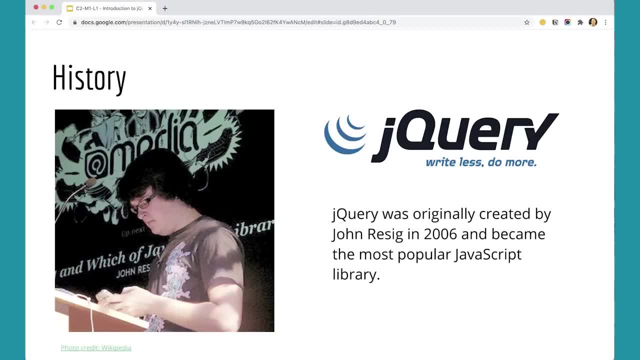 2006 and it became the most popular javascript library, and it's still a popular javascript library. in a recent survey, it was found that over 80 of websites are still using jquery. it's less popular today than it was back in the early 2010s, where it was at its height, but it's still an 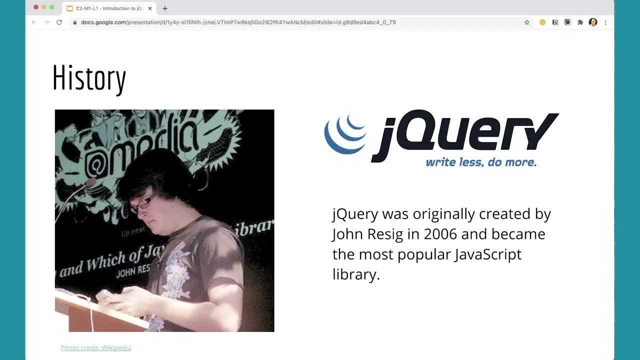 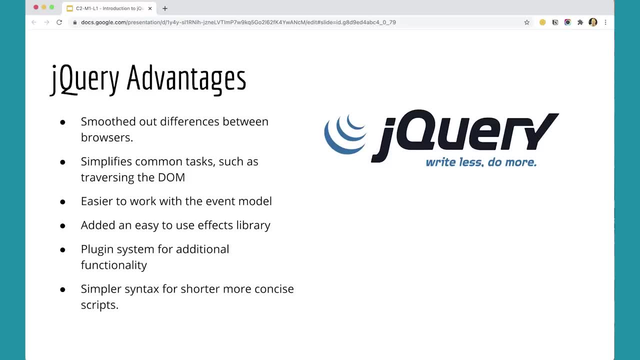 important tool to learn and good to know. there are some specific advantages that came with jQuery when it was invented, and some of these advantages exist today, but are they're somewhat diminished. but let's talk about them. first of all, it smoothed out the differences between browsers. back in 2006, when jQuery was invented, javascript was not implemented evenly across browsers and 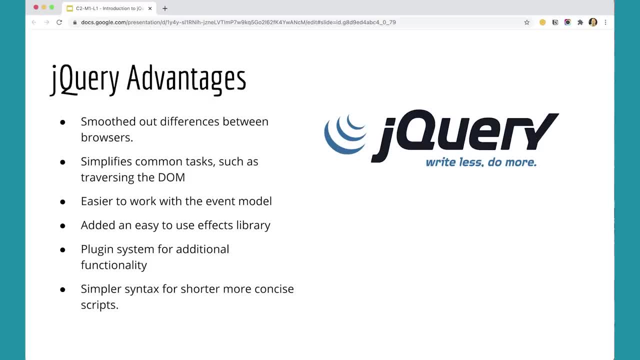 jQuery was really great at kind of smoothing out those differences from one browser to another. it also simplified common tasks such as traversing the DOM. it provided a lot of ways of getting elements on the pages that we didn't have with plain javascript back in the in the late 2000s. 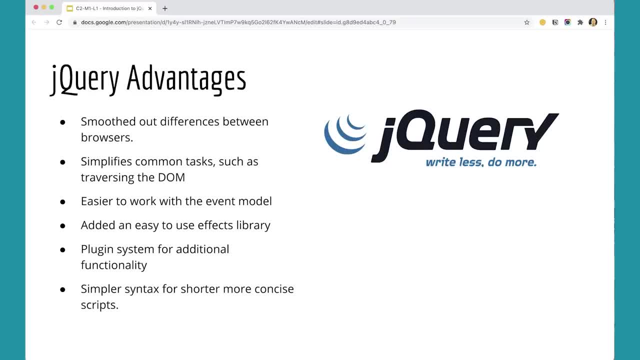 or early 2010s. it also provided an easier to work with event model for capturing clicks and scrolls and other kinds of events that users might use in the process of working with the page- events that users might trigger. so it provided this event model that was easier to access and easier to. 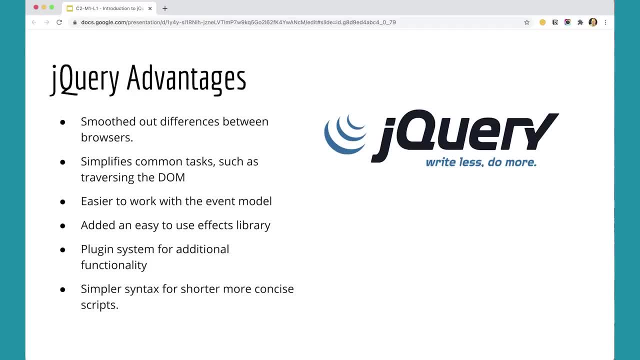 use, so it was easier to create interactive scripts that could hook into that event model in jQuery, and jQuery also provides an effect slide library that's very easy to use and really exciting and it's really kind of a cool effects library that provided a great way into programming, into creating interactive elements for a lot of for. 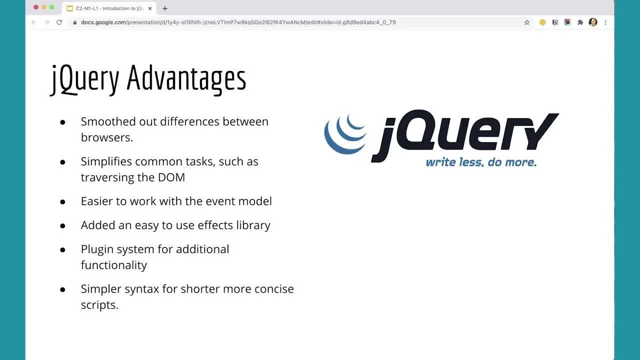 a whole generation of developers. then, on top of that, there's a plug-in system for additional functionality, so you could create plug-ins that added functionality to jQuery, and we'll take a look at this to some extent. and then, finally, last but not least, jQuery provides a simpler syntax and that 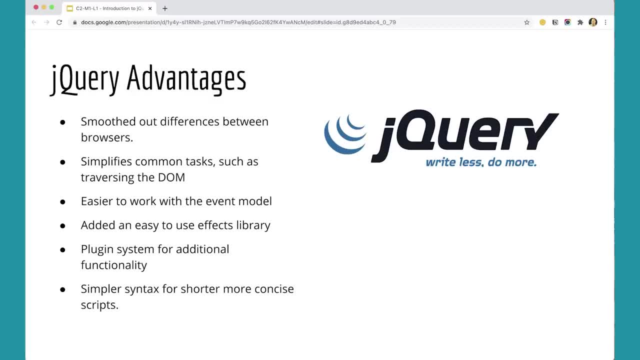 allows us to write shorter and more concise scripts, and these were all huge advantages to jQuery and contributed to making it the most popular javascript library. today, javascript jQuery is less useful than it used to be back in the early days, and some of the things that have that have sort of been smoothed over is that, remember in 2009, jQuery came out in 2006 and in 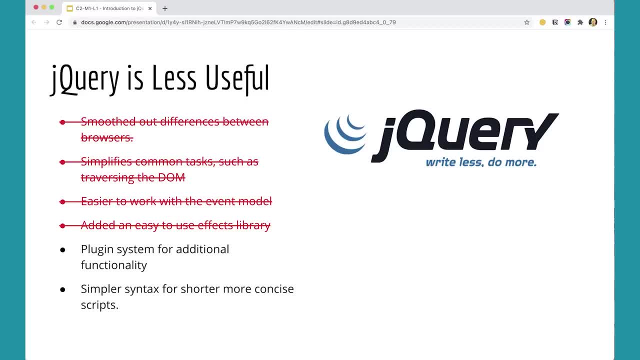 2009, the standardizing body decided to make javascript the scripting language for the web, and at that point, a lot of excitement poured into the javascript world and there was a a concerted effort from the people who were making browsers- web browsers like chrome and firefox- and 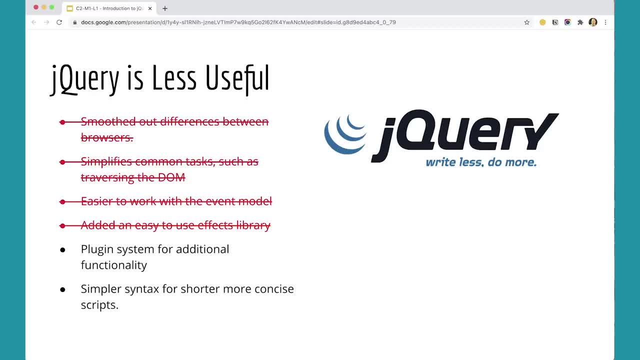 safari and internet explorer at the time. it's now edge, but for those companies that were making those- whether it was apple and microsoft or whomever- to standardize their implementations of javascript, and that really helped with with the development of javascript, plus the release of es6 or es 2015. 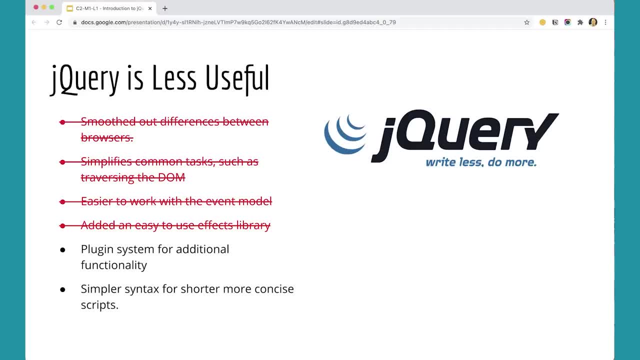 in 2015 really helped um with a lot of activity and a lot of effort, but it was a lot of fun and a lot of work for javascript and of the features of plain vanilla javascript so that we don't need as much from jquery as we once did. 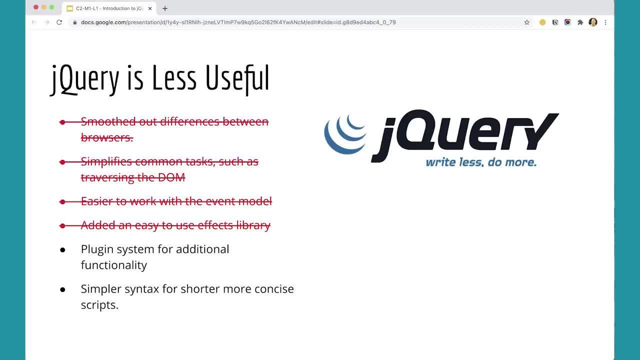 so we don't need to smooth out the differences between different browsers as much anymore. the implementations in different browsers- pretty much the same now- are very similar, so we don't need a lot of that anymore. in terms of simplifying common tasks such as traversing the dom, we've already explored query selector and query selector, all which are great tools. 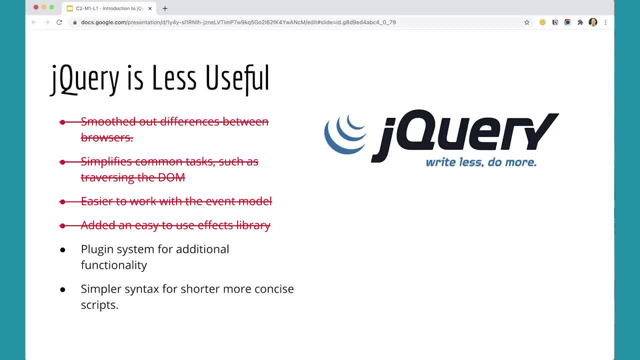 for accessing elements in your dom that are built into plain javascript now, and those have really helped minimize the need for jquery to do that kind of thing. also in plain javascript we now have the add event listener method, which is great for adding event listeners for all different types of events that users might trigger or might be triggered by the system. 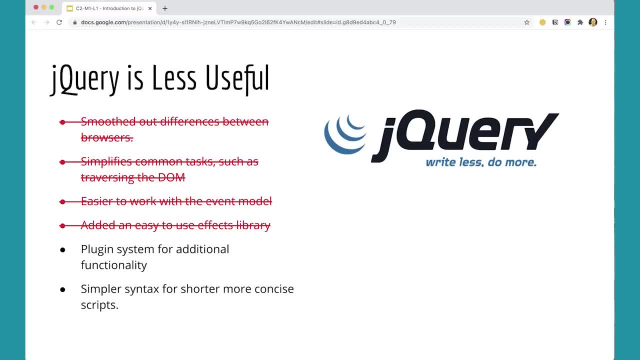 so using using that event listener model sort of limits the need for the easier to work with event model that jquery had to offer. the effects library is interesting. the jquery effects library is great and it's really great to work with and it's fun to work with and it's still useful from time to time. but these days we would much prefer to. 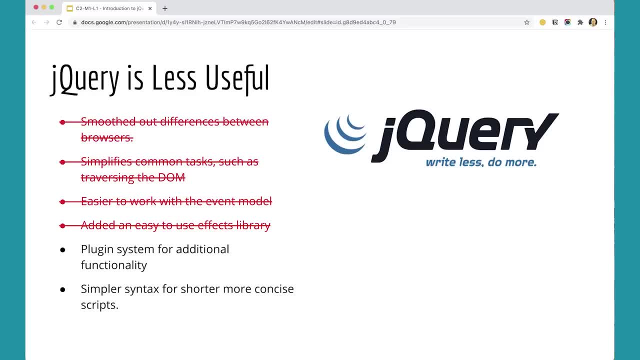 use css to create animation, because css will take advantage of the device's gpu, the graphics processing unit, as opposed to the cpu, the central processing unit, and that will make your animation smoother and work better, especially for older, slower devices, these kinds of things- phones, older phones, this kind of stuff that you know the jquery animations will feel a little bit clunky. 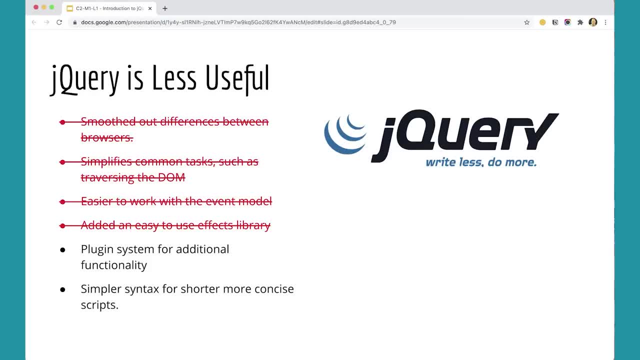 because jquery is using javascript to create those animations. so the effects library is not as useful today as it once was, although it can still be used useful. the two things that are still really useful about jquery are the plug-in system for additional functionality. there are thousands of plug-ins written for jquery and we'll look at. 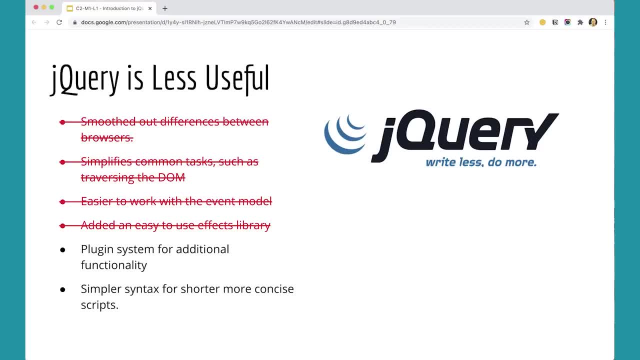 a few of them, but you can explore many on your own, and the wonderful thing about plug-ins is that other people have written a whole bunch of code and you can take advantage of that and build all kinds of cool things from the code that others have written, and that also helps. 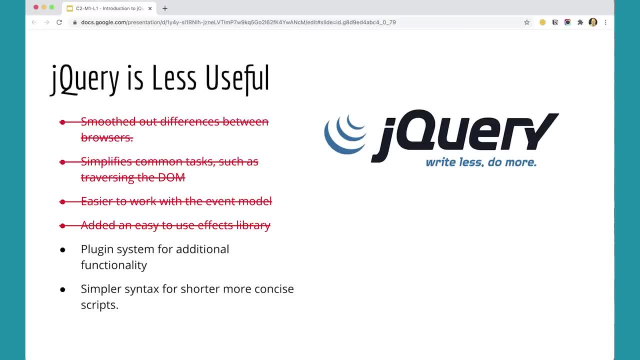 prepare you for other types of libraries of code. if you get into node and npm and these kinds of things, doing this stuff with jquery will help sort of prepare you for that world. the simpler syntax for shorter, more concise scripts is also still true. it's perhaps less 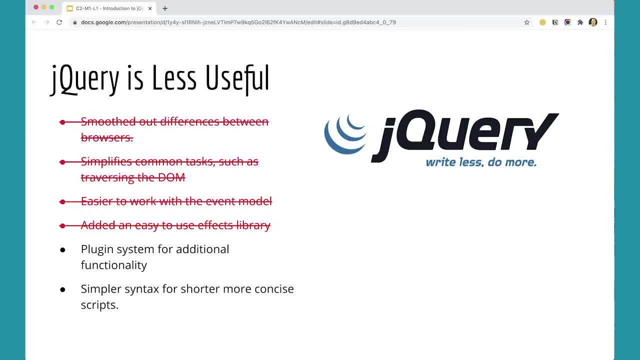 true than it once was, but it's still true. you'll see, we'll do some exercises and some examples where you'll see that the scripts are shorter and more concise and if you're just learning programming first time, that can be a way into programming. it was a way into programming for a lot of people. 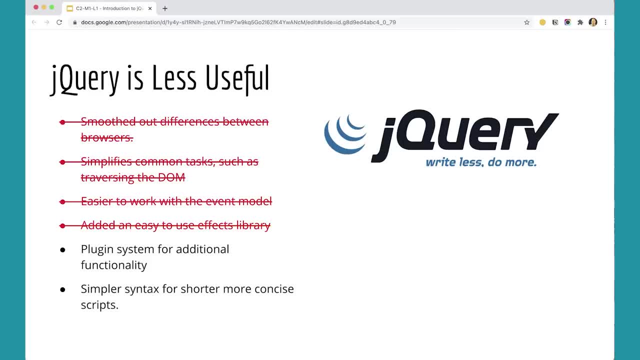 who got into javascript in jquery back in the day. it certainly was for me personally where i wanted to do something that was fun and interactive and i could write fewer lines of code with jquery than with javascript, so that was a real bonus for me as i was learning javascript back in the day. 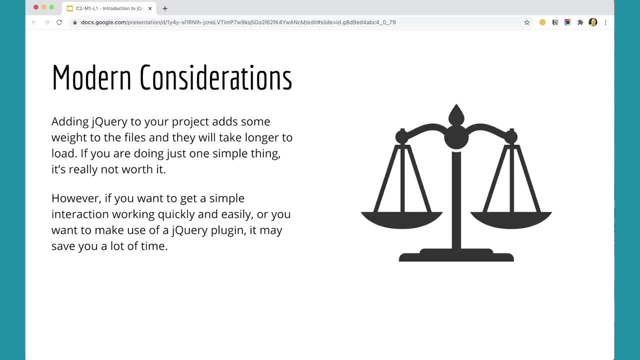 there are a lot of modern considerations to take into account when deciding whether or not to use jquery. adding jquery to your project adds some weight to the files and they'll take longer to load. and if you're just doing one simple small thing, it's probably just not worth it to load jquery to do. 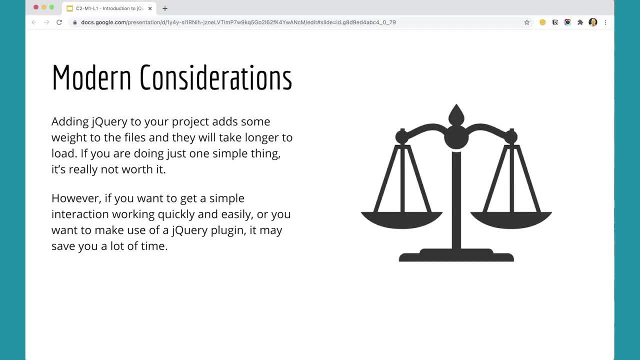 that, however, if you want to get a simple interaction working quickly and easily, or if you want to make use of a jquery plugin, using jquery could save you a lot of time and really be worthwhile. so you have to really consider it on a project by project basis. 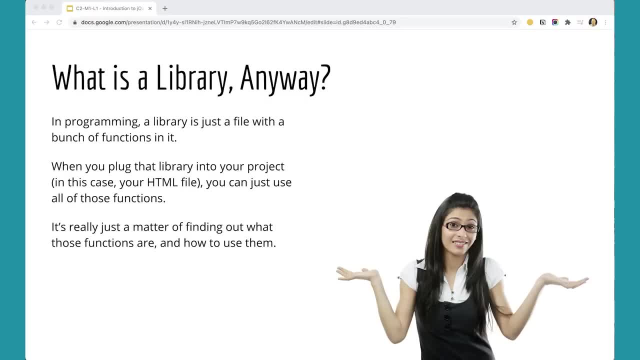 what is a library anyway? in programming, a library is just a file with a bunch of functions in it, or it could be multiple files that you link up to your project. in this case you'd link to that, link them into your html file, and then you can just use those functions if you're. 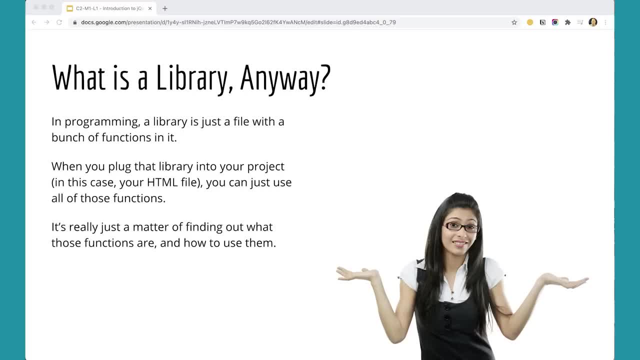 familiar with a lot of programming and you haven't done a lot of this kind of thing. it may seem like a unusual or a new concept for you, but just think of it as something as simple as that. it's just a file with functions in it that you can access and use in your project. 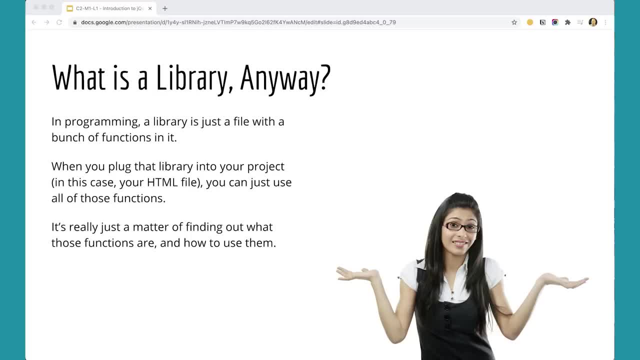 and then, once you've linked it to your project, it's just a matter of finding out what those functions are and how to use them, and that's really how jquery works. it's a file that you can add to your project, and when you do, you have access to all the jquery. 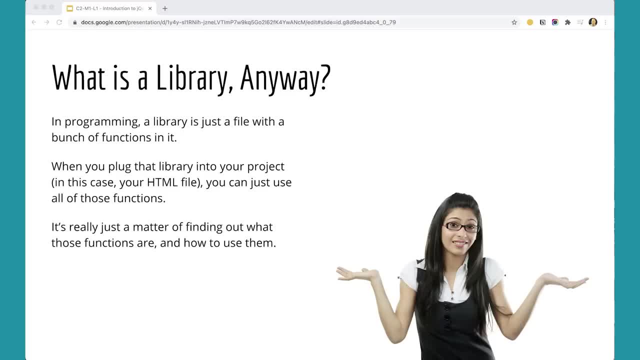 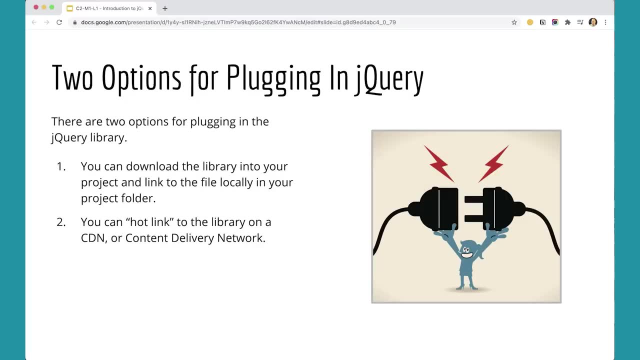 and all the functions that come along with jQuery. There are two options for plugging in jQuery. The first is you can download the file, the actual jQuery library file, and put it in your folder with your other JavaScript files or other files for your project, and then 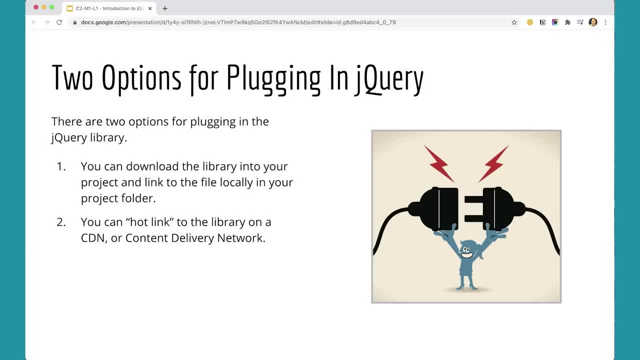 link to that file locally in your project folder And then when you load your web page, it will load that file along with all your other files. Or you can hot link to the library on a CDN or a content delivery network. So what that means is, instead of putting the file in your project folder, you're actually 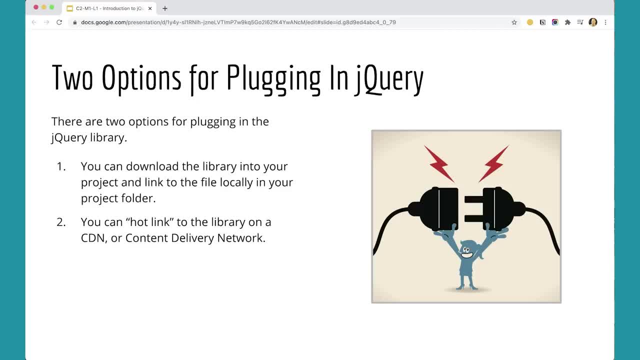 linking to the file already out on the internet And a CDN or content delivery network, means that when you do that, you'll actually be getting the file from the closest server to you. A CDN has servers all over the globe and when you go to load a particular web page, 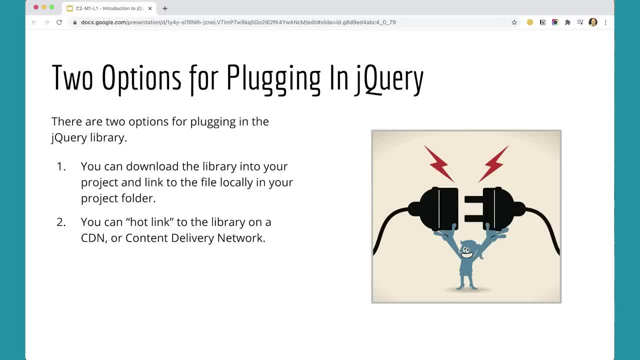 it's looking at your IP address and figuring out where you are and then getting the file from the closest file server so it will get it the fastest that it can. So there are both these ways of getting jQuery into your project and we're going to look. 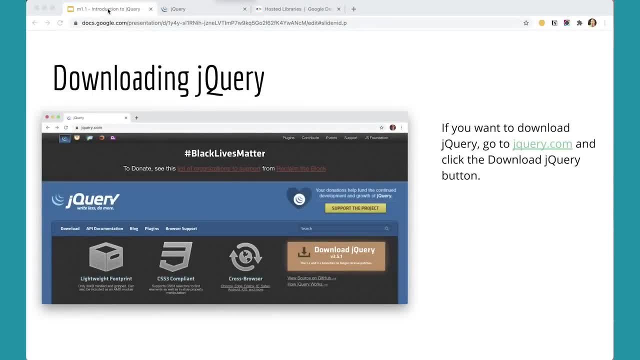 at both of them. First, we'll look at downloading jQuery. Okay, And to do that you can go to jQuerycom, and I have that website pulled up here and you can click the Download jQuery link. So let's go over here. 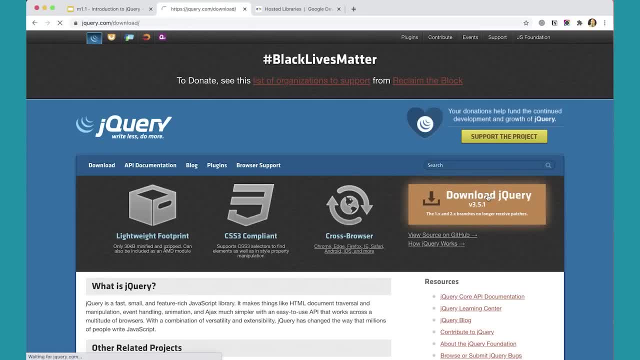 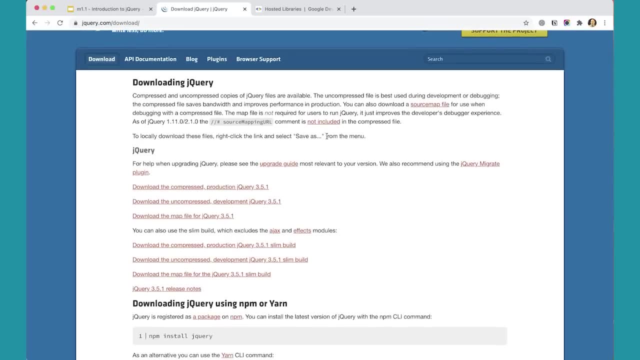 And I can click on Download jQuery here And that will take me to a page that, if you're not used to doing this kind of stuff, will look a little confusing, because we've got a whole bunch of links here and it's not. 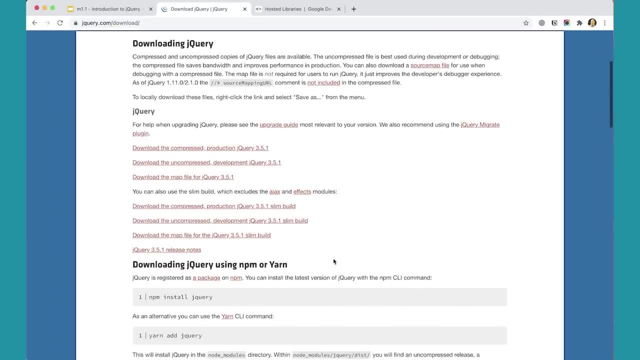 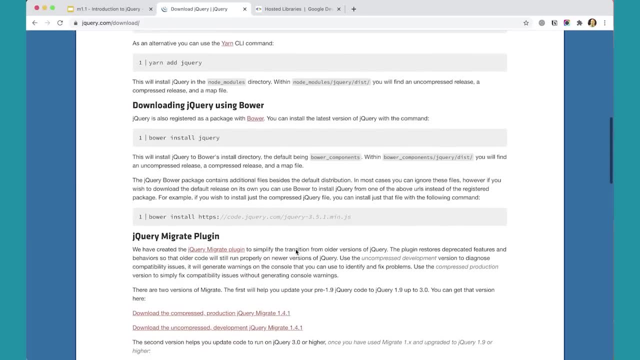 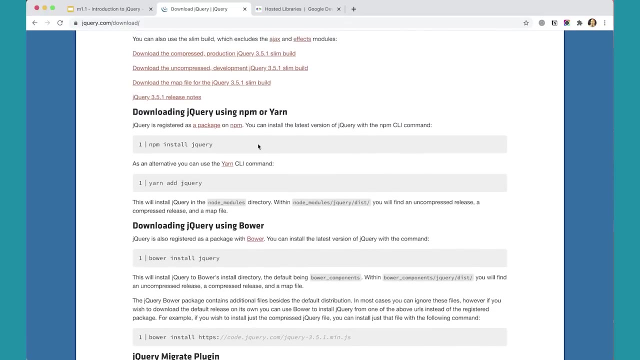 really clear exactly what it is you should actually be downloading. And then they've got this stuff with NPM and Yarn and Backup And this Migrate plugin and you know all this other stuff on the page, So it can be a little bit confusing. 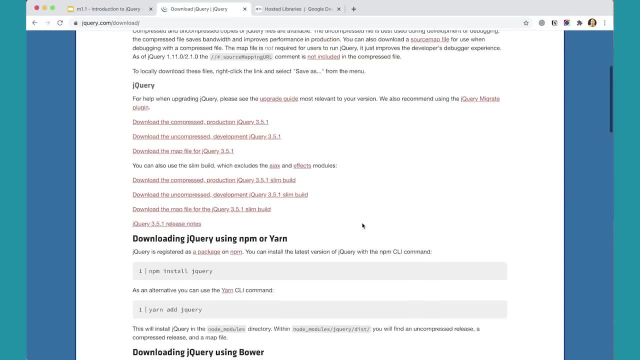 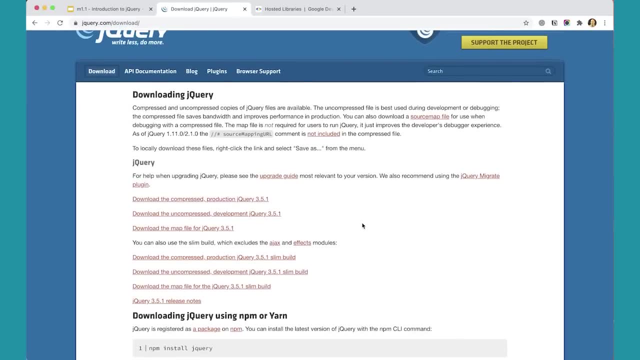 The NPM, Yarn and Bower are all build tools that you might be using if you're in a particular environment that's using these build tools. But we're just going to download the actual library file itself, and what we want is the 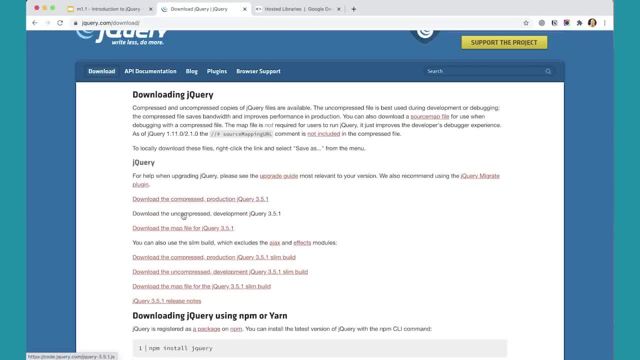 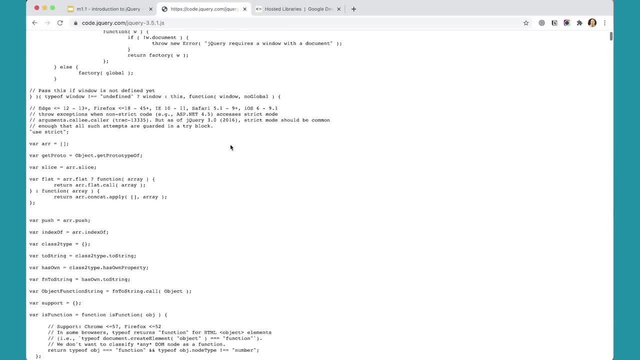 compressed version. There will be a compressed version. There will be a compressed version. There will be a compressed version and an uncompressed version. The uncompressed version will look like this And it looks kind of like JavaScript that you've seen before with bar and all kinds. 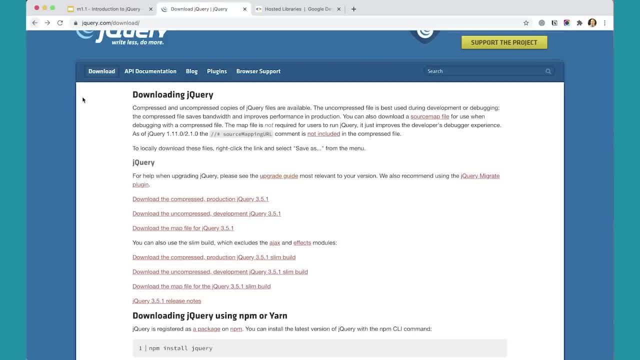 of all this kind of stuff. The compressed version is going to remove all of the white space and sort of compress it down, so it's not really made for human reading at all. It's made just to be loaded on your computer, But it'll be smaller. 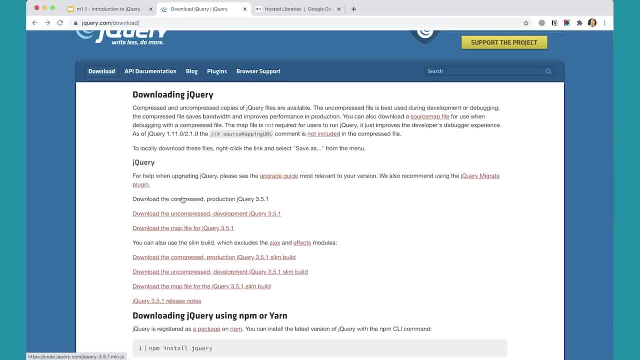 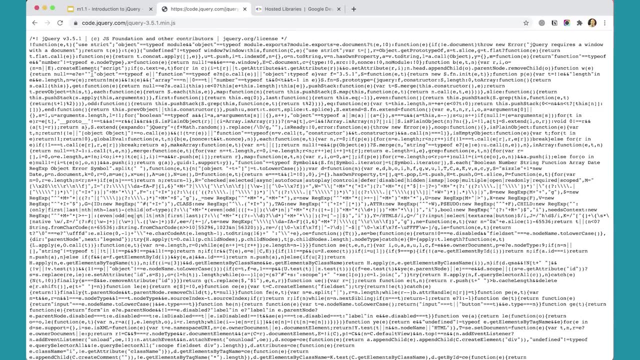 It'll be a smaller file to download, And so what you want is the compressed production version of jQuery. So if you click this one here, you'll get something like this And you can see up here. it says: jQuery version 3.5.1.. 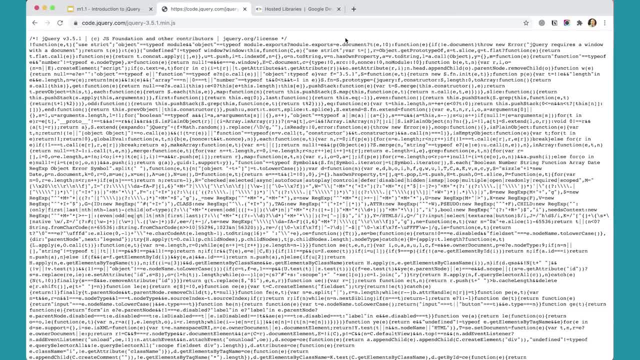 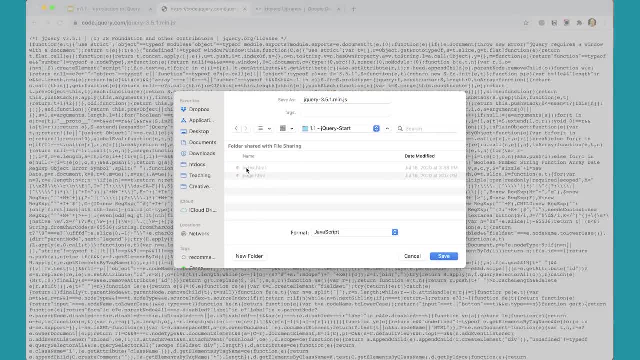 Okay. So to download this, if you just right click in the white area here and do save as- and I'm going to save it in my downloads into my jQuery start folder and that's where you should put it as well. So I'm going to just put it in here and save this. 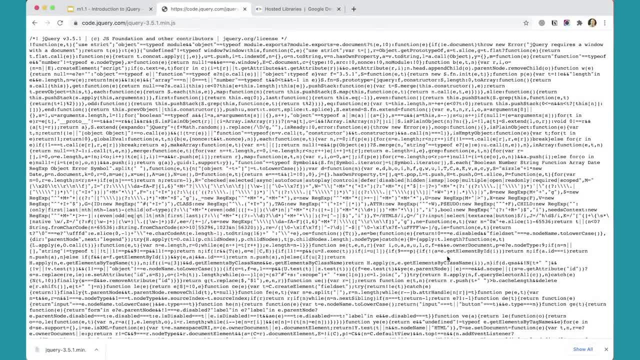 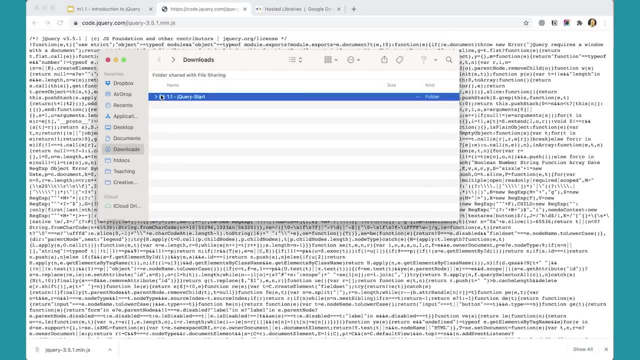 And I'm going to save it in my downloads into my jQuery start folder- And that's where you should put it as well, So that now I have a copy of jQuery in my jQuery start folder here. Here it is: jQuery 3.5.1 min is the minified version that's been compressed in. 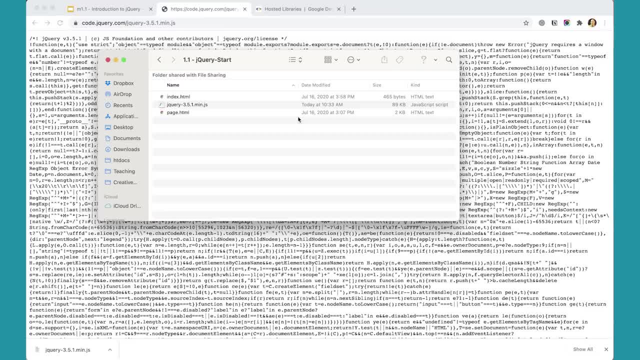 And generally you want to get the minified version so that it's- and you can see here it's- taking up 89K on my drive. Just for fun, let's see how big the other one is. We want to see how big the other one is. 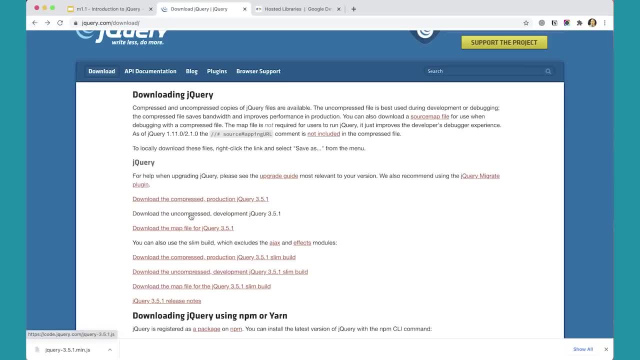 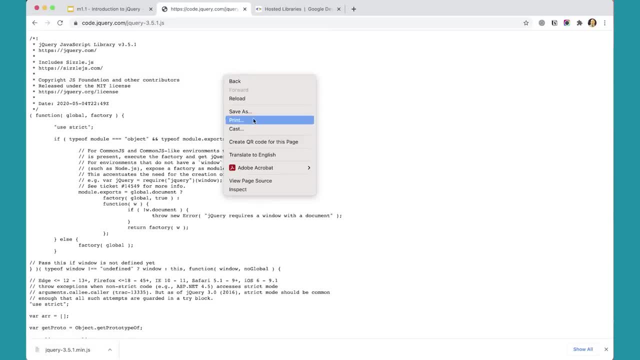 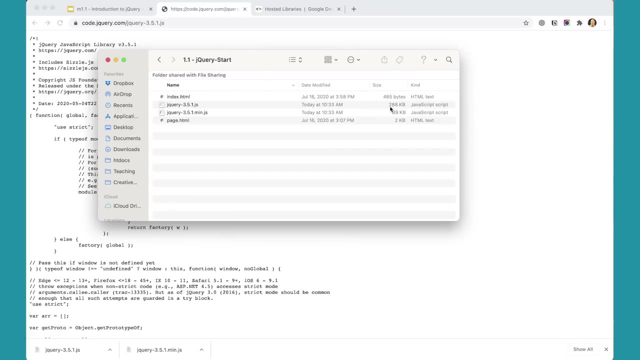 If I right click and choose save as and download this one and then come back and look at this, You can see this one is 288K. This is a lot larger. This version here is the size of maybe a medium size image on your webpage. 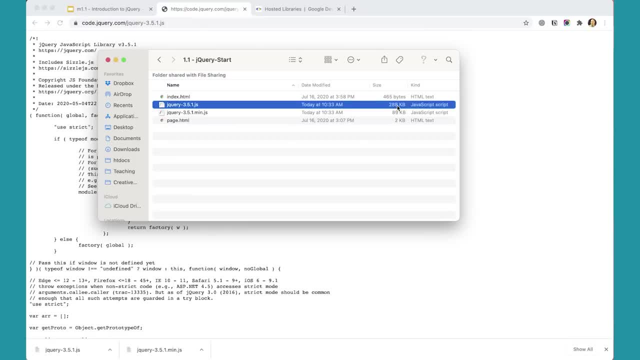 It's not that big. this is significantly larger. it's going to take longer. if you use this version in your project, it's going to take longer for you to download this. so you might be asking: well, why do they provide this? well, if you wanted to go in, if you were an engineer and you wanted to go in and mess with, 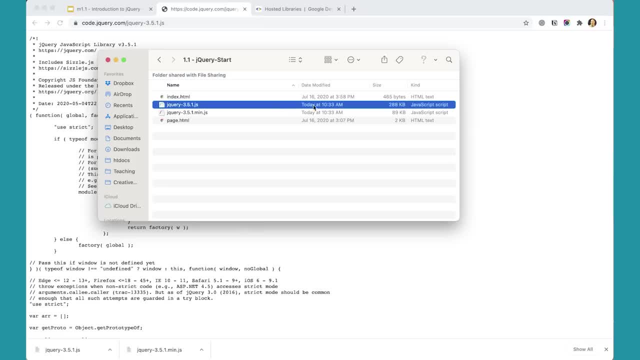 jquery, create your own fork of it. you could. you could actually do that here, but we don't really want to do that, so i'm just going to delete this version. we don't need that at all. we just need the unified version weighing in. weighing in at 89 kilobytes: okay, great. so now we've got jquery. 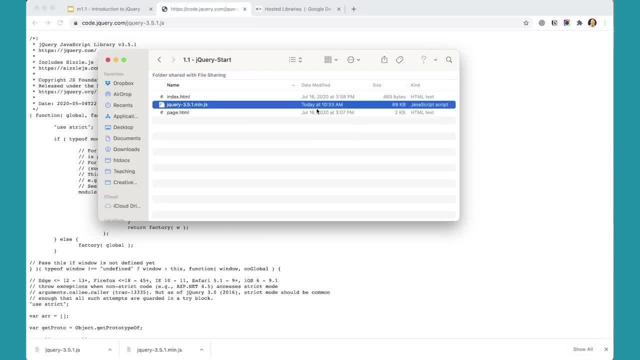 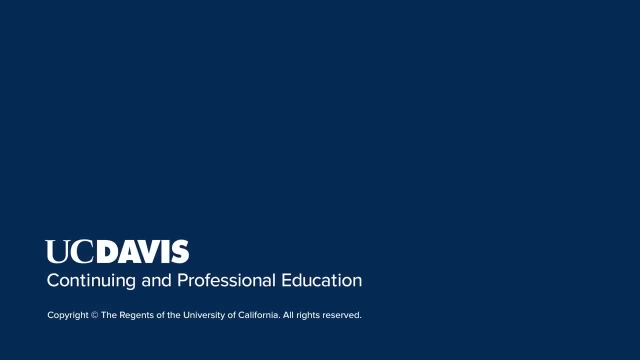 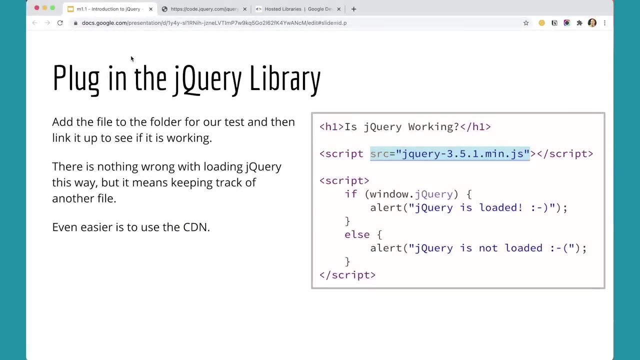 let's get it plugged into our, into our html file. we'll plug it into our html file here, plugging in the jquery library. so now we've downloaded jquery. all we need to do is add it to our jquery library. so now we've downloaded jquery. all we need to do is add it to our. 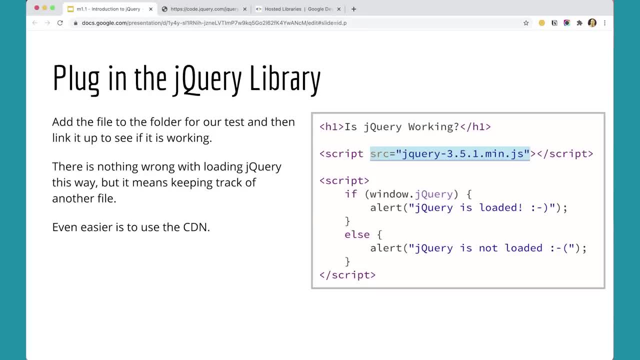 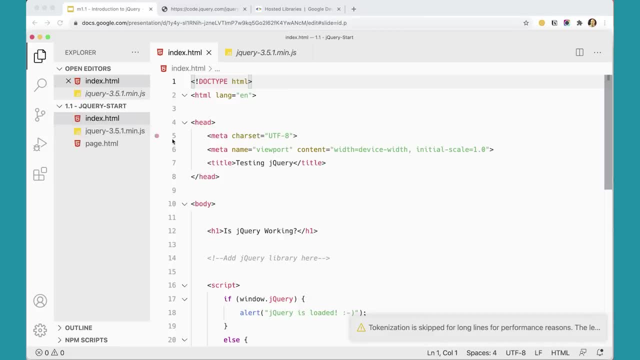 file and i have those files open in my visual studio code here. so this is the same files as the file i just downloaded here. so there's jquery and i want to go ahead and add jquery to my file here so i can come down here and i can add a script, tag, script and what i'm going to put in. 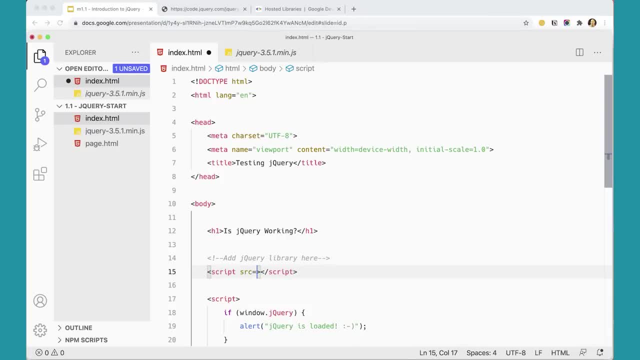 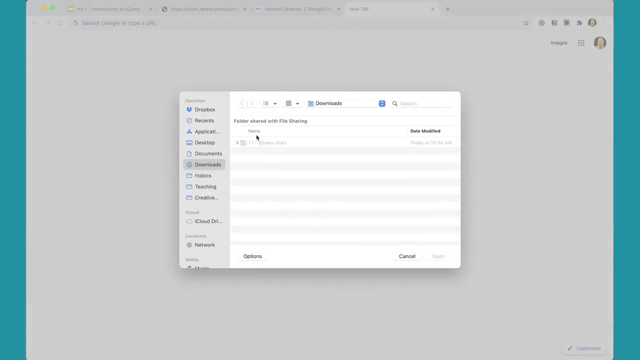 here is source: src equals quote, and then i can actually just pick this file from the list here and there we go. so now jquery is plugged in and if i test this file over here, i come over here and open a new tab and do open and go into my jquery start folder and open this index file. it'll pop up. 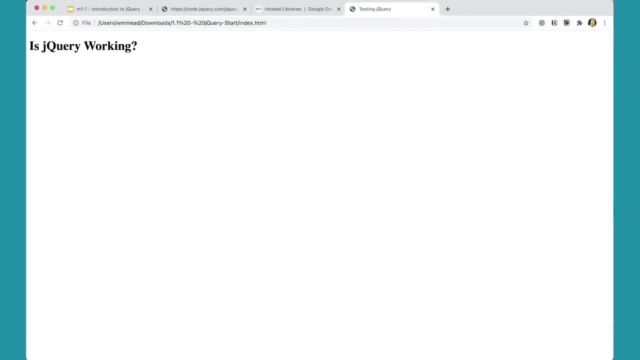 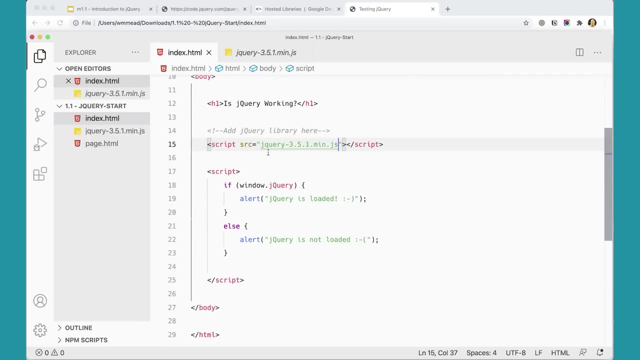 and it'll say: jquery is loaded. if i were to remove that script- so down here you can see if windowjquery alert jquery is loaded- if i were to remove this script, suppose i comment this out just for a minute and save this and then come back and test it. it'll come back and it'll say jquery is not loaded. 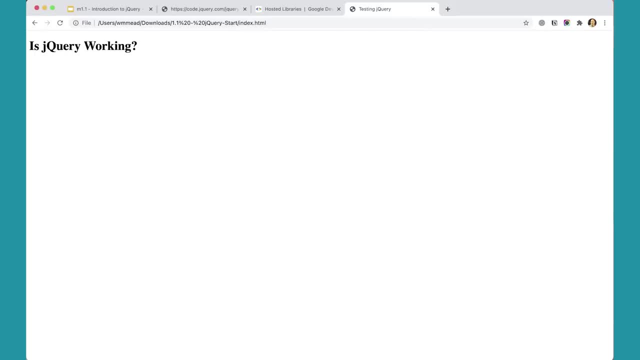 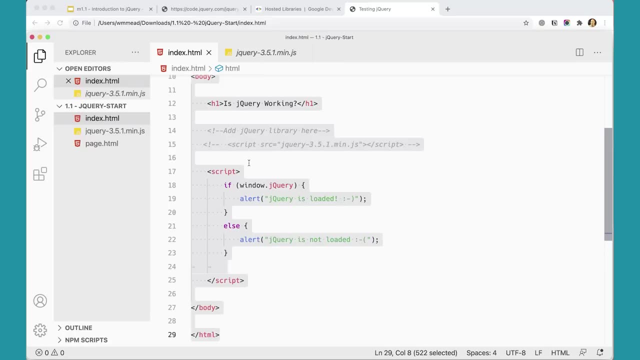 so, in order for this script to run, it requires jquery, because we're testing to see if jquery is here. so, um, oops, there we go. so now jquery is loaded and, um, this statement is true and we're getting this alert box. so that's great. so we can load jquery by linking it here and, you know, downloading it and putting. 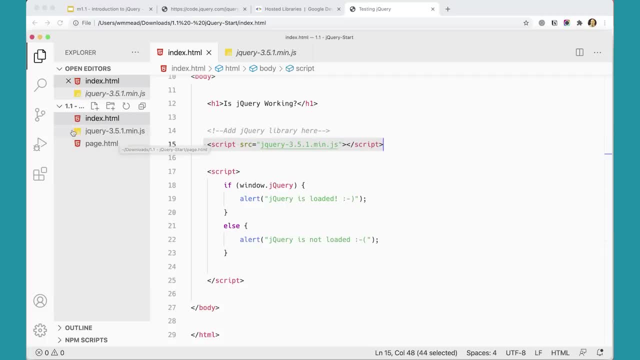 it in our files and linking to it. when you do it this way, you have an extra file to keep track of. you have to keep track of this jquery library file and make sure that it doesn't go missing from all your folders and files. not that big a deal, but it's one more file to keep track of. 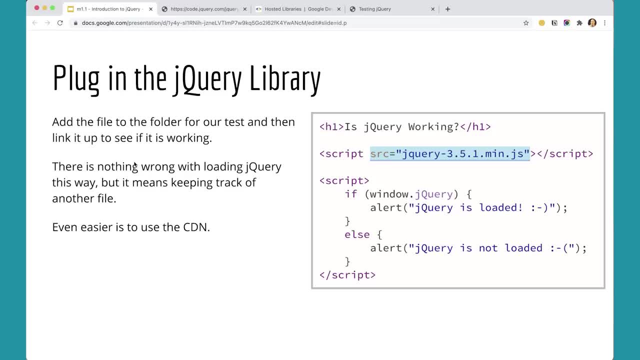 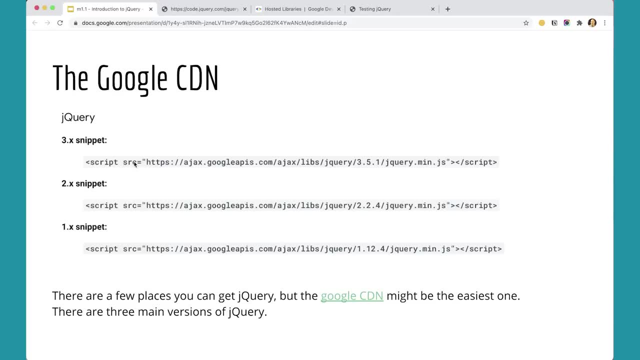 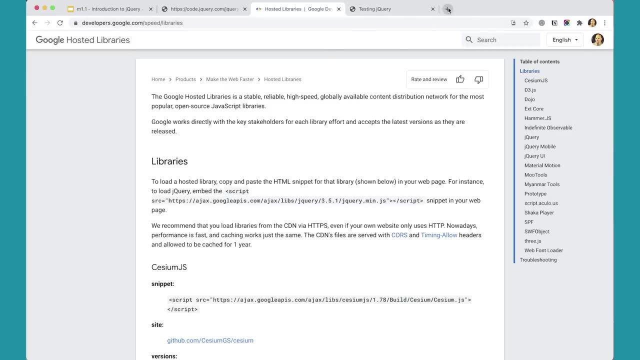 even easier is to use a cdn to load jquery, and the cdn i prefer to use is the google cdn and i have that pulled up over here, and if you want to get to this cdn, the easy way to get to it is just to google google c. 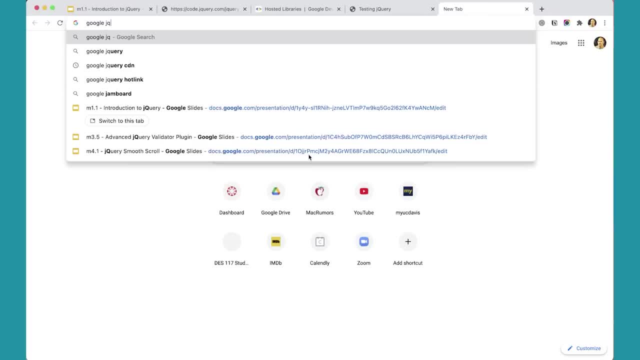 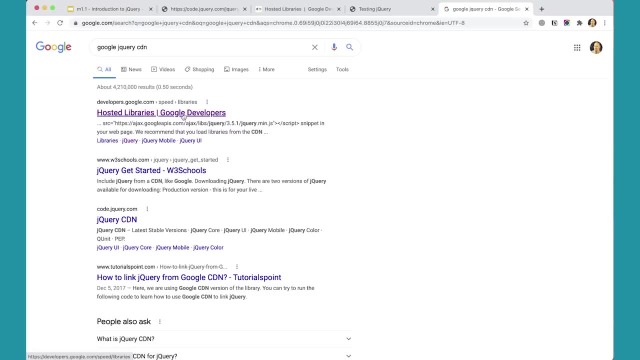 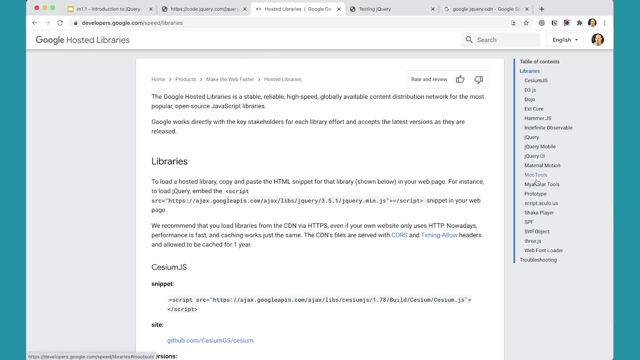 jquery, i can type cdn. there we go and you'll see hosted libraries on google. so that's this link right here, and over here they've got a lot of libraries that you can access through google that they host on their cdn. one of them is jquery, so we can actually go to this link. 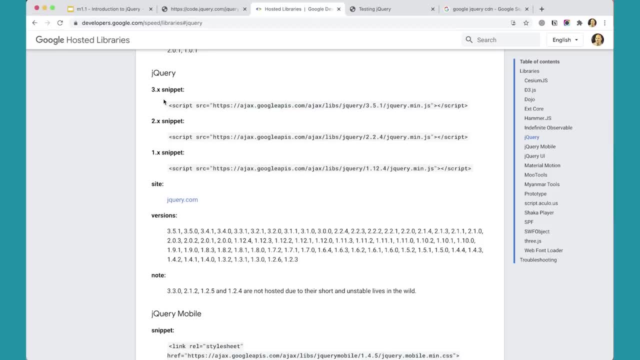 here to jquery and you can see that jquery has three different versions, three sort of flavors of jquery that include different features. the version 1x snippet is the oldest version of jquery and it's loading 1.12.4. so this is really the 12th version, 12th major version of version 1. 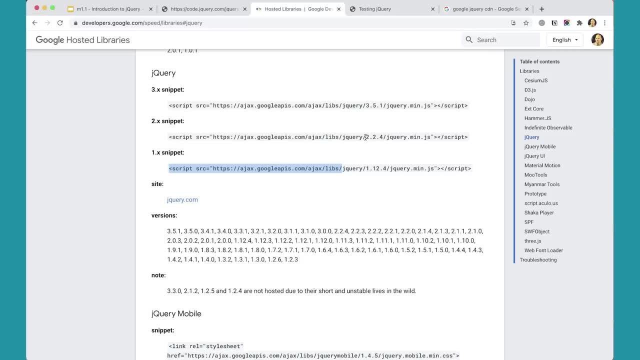 essentially. and then we've got version 2.2.4, which is the second major version of version 2, and in version 2 they did a number of things, to you know. they removed support for ie6 because they basically got away at that point, you know. so they've done some different things in these. 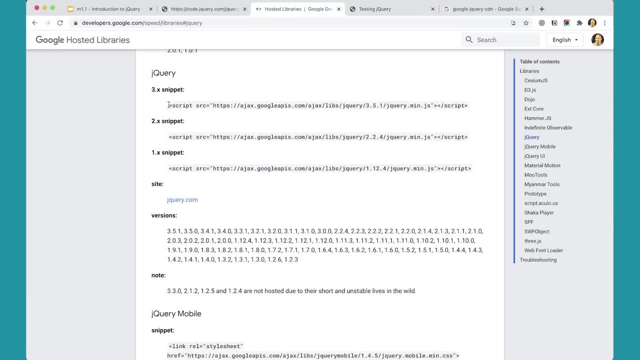 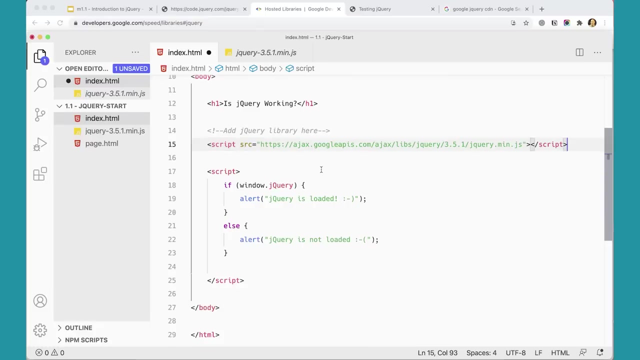 different versions. the most recent version, the version that we downloaded, is version 3.5.1, so to get the same one that we had before, you can just copy this entire script line here: oops button there. there we go, copy that line and go back to our file here and paste that line in instead. 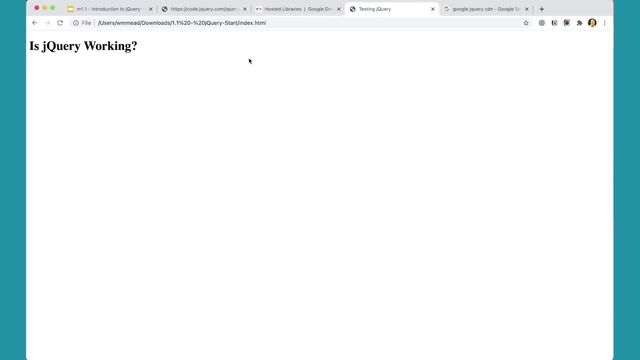 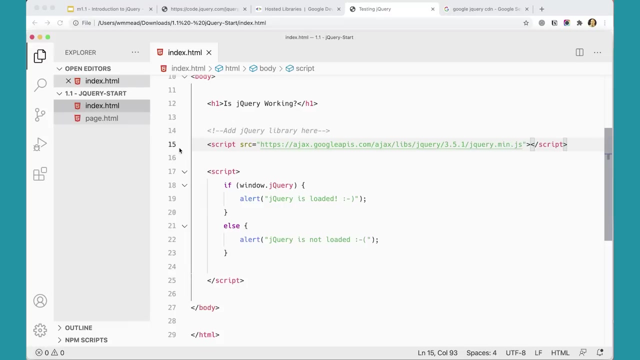 and you'll see if we save this and come back into testing jquery. jquery is loaded, so instead of loading from the file that i have locally here, i can now delete this file and it will work just fine. delete now that file is gone, and but this will work just fine, because it's actually going to load from the file that we have here, so we can. 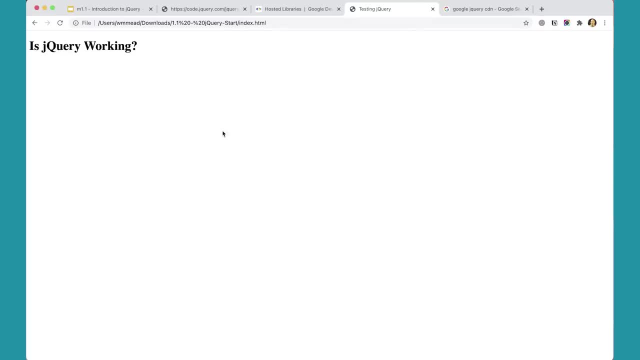 actually load jquery from the internet. of course, if the internet's down it's not going to load it, but if the internet's down you need to get to your web page anyway. so so it's a little bit easier to use the cdn to load jquery, because it's just one less file to have to download and keep track of. 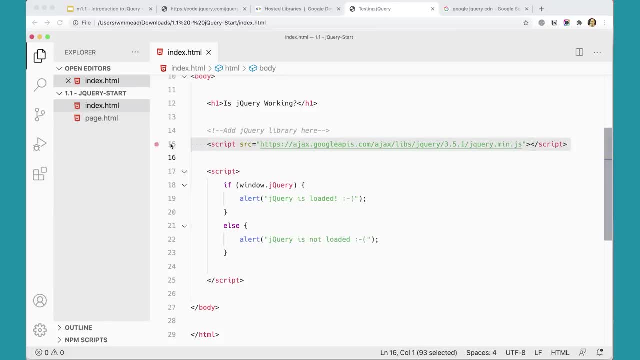 so usually we will be using this method to load jquery and there are times when you might want the older versions. generally we'll use the newer version of jquery, but we're not going to use the newest version. but you might want the older versions if you're using a function or a method. 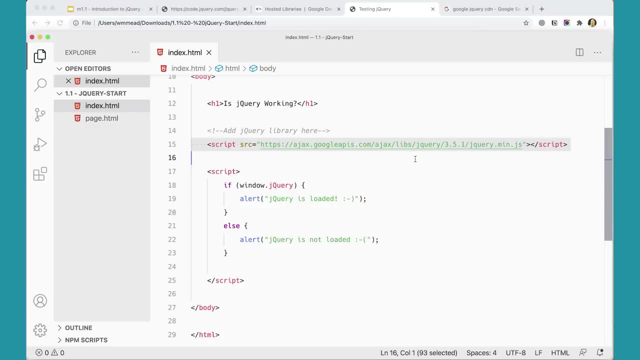 in jquery that has been deprecated, or if you're using a plugin that was built using an older version and it needs some functionality from the older version in order to work. but generally, generally, we're going to use the newer, newest version of jquery- version 3.5.1 at the time of 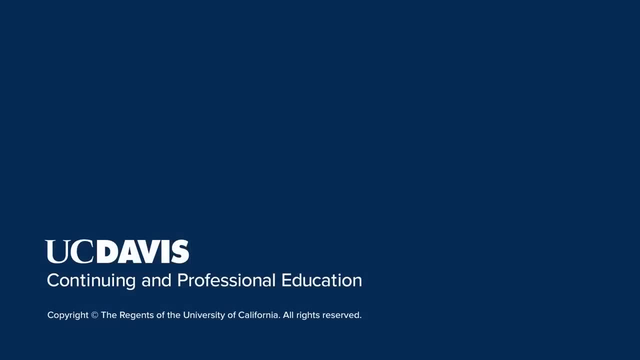 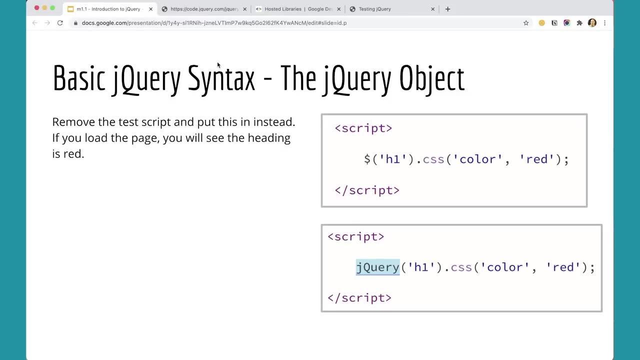 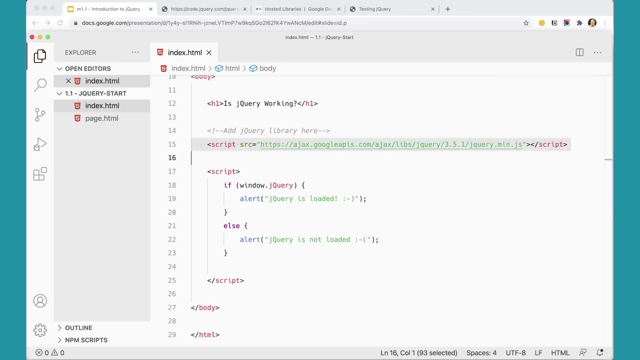 this recording. so now that you have jquery working, let's do something with it. do something more than just to show that it's working and we'll use the same file. we're just going to replace the script on there, so just so we can see that something is happening to our actual web page. so if we come, 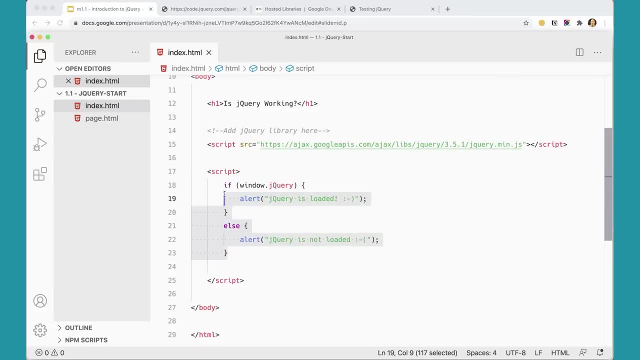 back over here. we can get rid of this if l statement, just delete that for a moment and let's put in a jquery statement. so try this out. so instead- and i'm just going to there- we go dollar sign. we're going to go get the h1 on the page, which is this element: here is jquery. 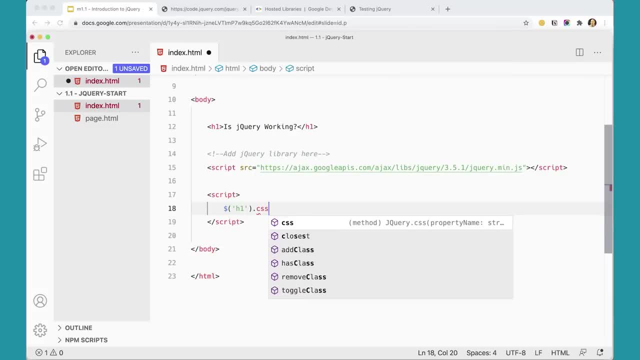 working and we're going to use the css method in jquery, like that, and what we're going to do is we're going to set the color of the h1 to red. So if we just do that, just do this one line and then save it, and then, if you come over, 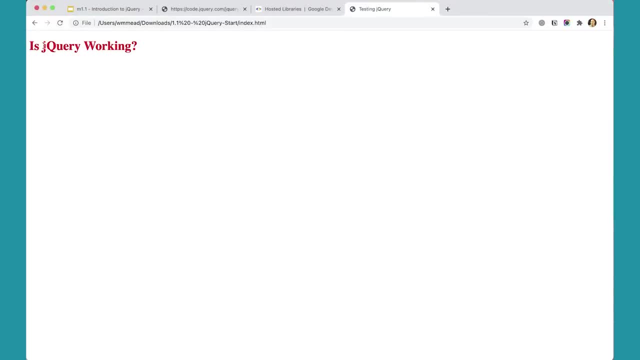 and run this testing jQuery again, you'll see that it turns the h1 red here. If I inspect this element here, you can see that what jQuery has done here is it set the style color red on the h1.. Now, before we did the same thing with querySelector or querySelectorAll, we've done this kind. 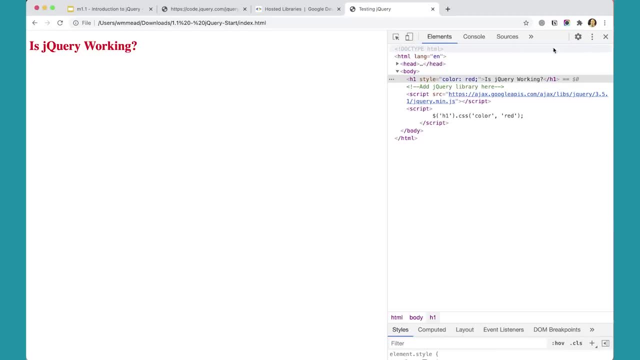 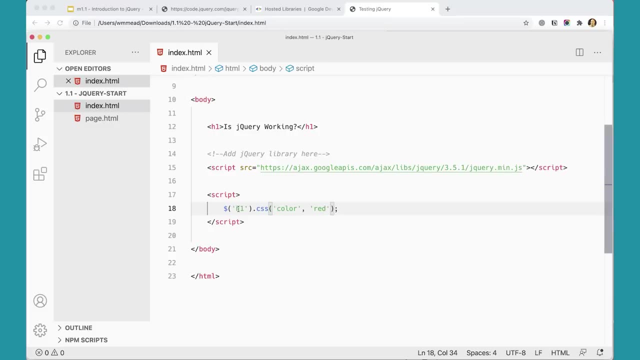 of thing before in previous lessons, but now we're using jQuery to do it, And in jQuery you can see we have just a really simple syntax here that uses CSS style selectors to access elements in the page and we've got methods that we have access to, because 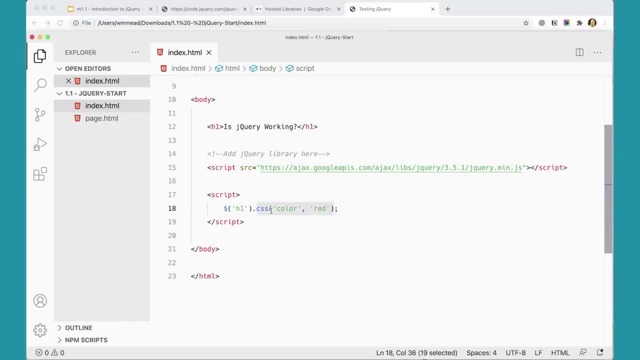 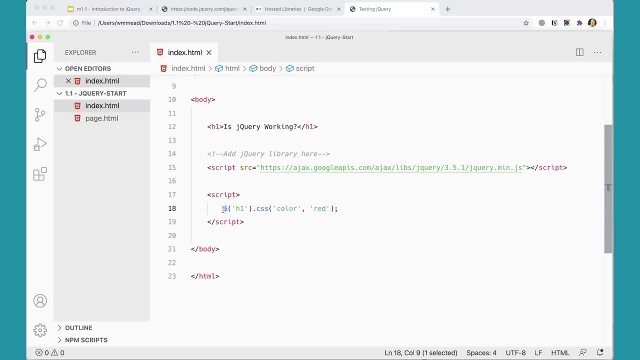 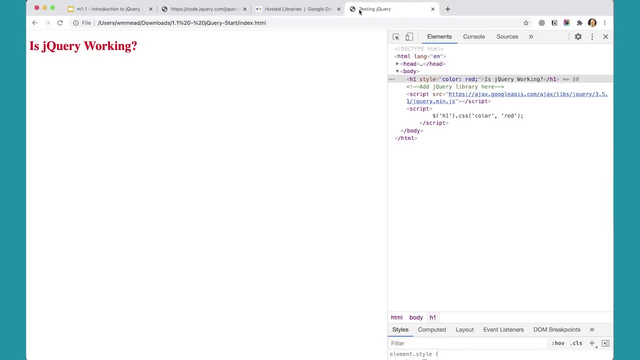 jQuery library and you can go to the jQuery library and you can go to the jQuery library. If you're wondering about the dollar sign here, the dollar sign is just a shortcut for the word jQuery, So I can put the word jQuery there and over here. this will run just exactly the same way. 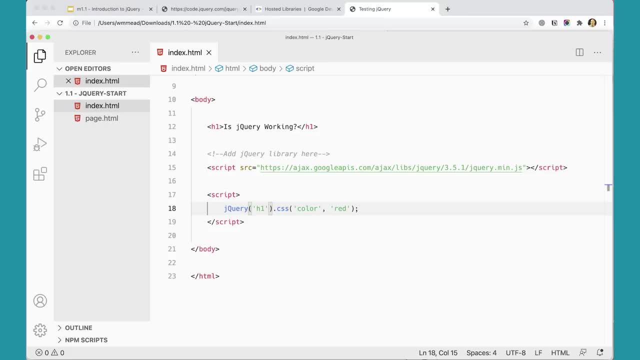 It'll work fine with using the word jQuery instead of the dollar sign, But generally we use the dollar sign as a shortcut just because it keeps our script shorter. it's less typing and you know why type all of these things, Why type all of those extra characters if you just type one? 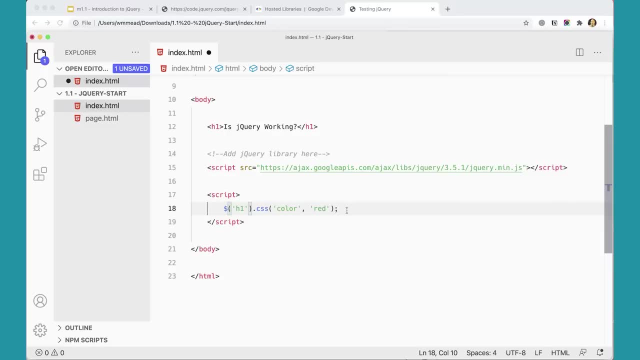 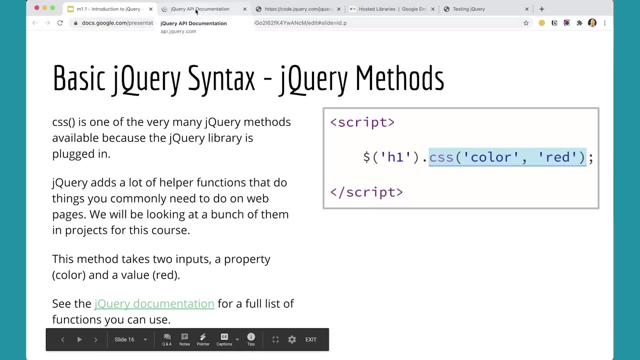 So we can put the single dollar sign in there. for that reason, This CSS method here is just one of a great many that jQuery has to offer that will help us affect our web pages And you can come back here. you can click on, you can go and look at the jQuery API. 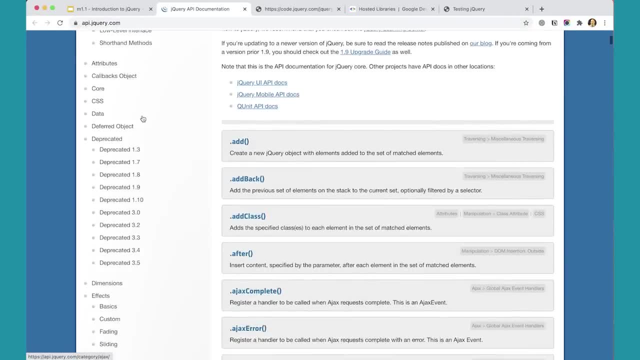 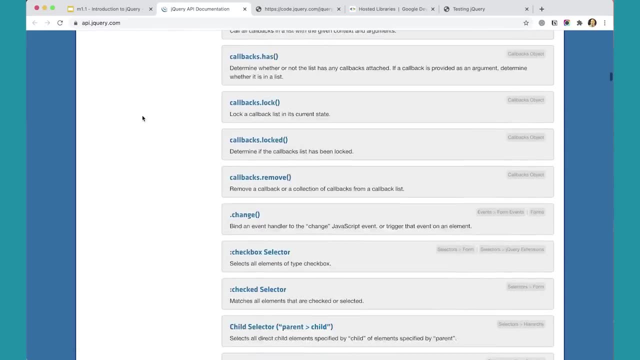 application here, and I'll put this link in for the lesson so you can access it easily. You can see that there's just tons and tons and tons of different methods that you have access to. as we go through and look at all of these, 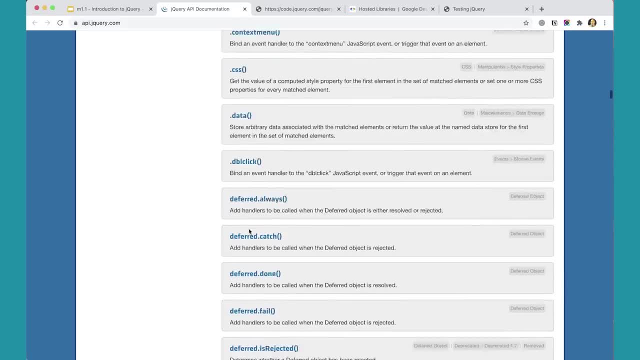 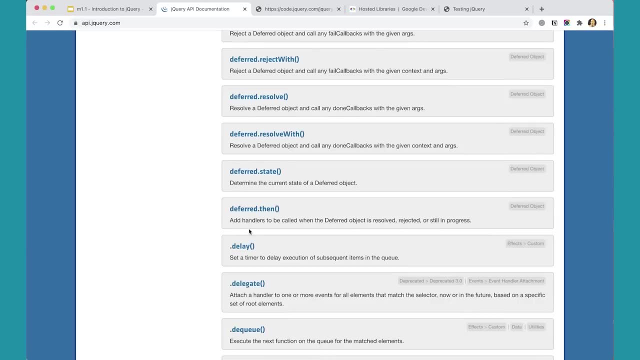 So here's the CSS one that we were just looking at, But there's tons of them in here, And jQuery gives you access to all of these different methods, So it's like having a kit that you can use to build things for your web pages just by. 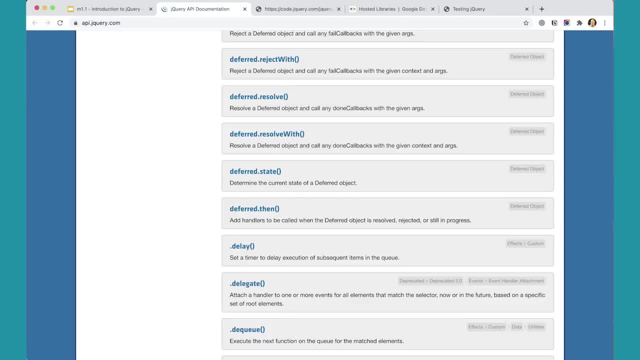 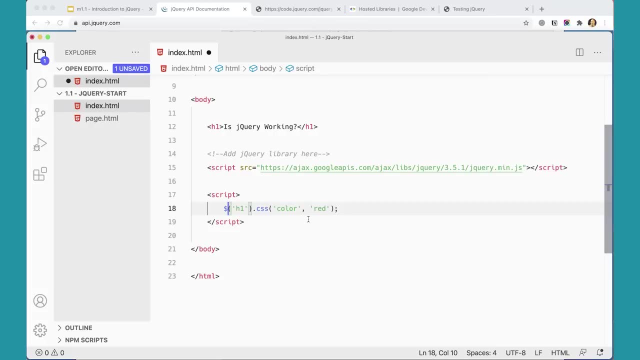 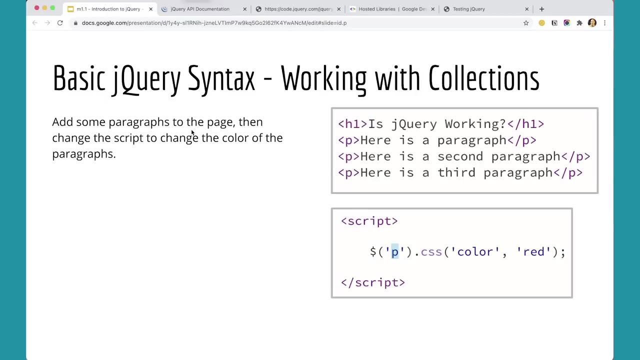 plugging them in and plugging in jQuery and then using these methods in accordance to the way they're described in the documentation. So let's try something else here. If we come back here and try, let's try adding a few paragraphs. 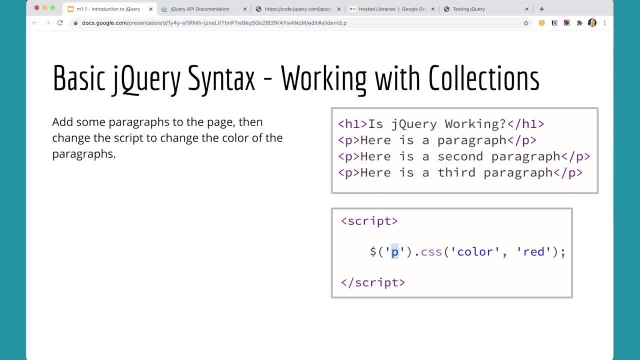 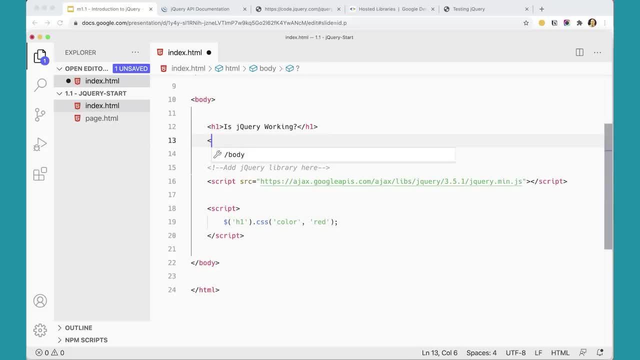 So let's just add a few paragraphs, And one of the nice things about jQuery is it allows you to work with collections of things. So if I come in here and just add a couple of paragraphs to the page, Okay, And I'm just going to copy that and paste it and add a few more here. 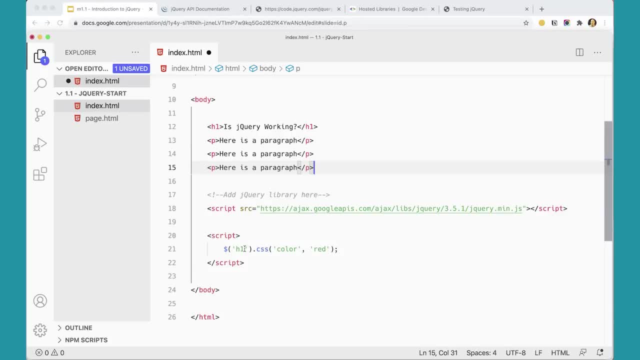 So now I've got three paragraphs on the page Now down here, if I change this to p. if we were doing this with plain JavaScript, we would need some sort of loop because we would do querySelector all Or getElementsByTagName or some method like that which would give us an array of items. 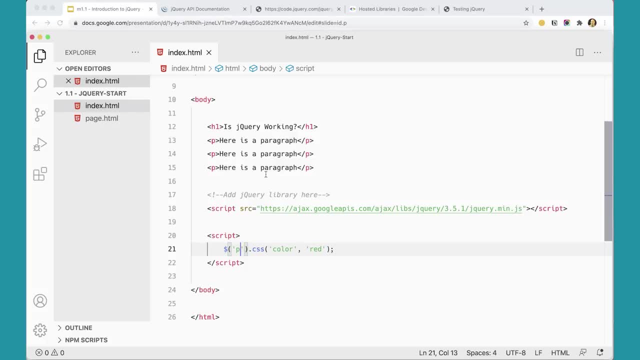 that we would then have to loop through to turn them all red, And we've done that before. We've done that in some of our previous lessons. So, but here with jQuery, one of the things that makes jQuery shorter and more concise is it'll work with groups of elements. 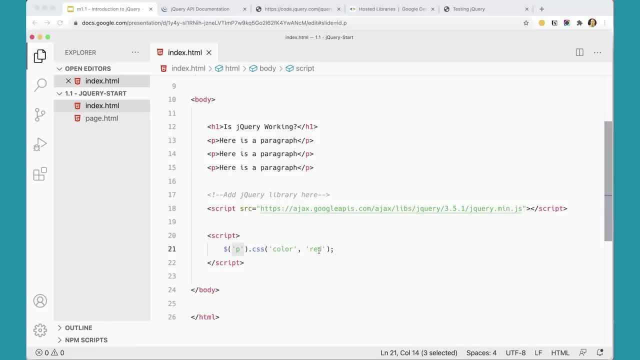 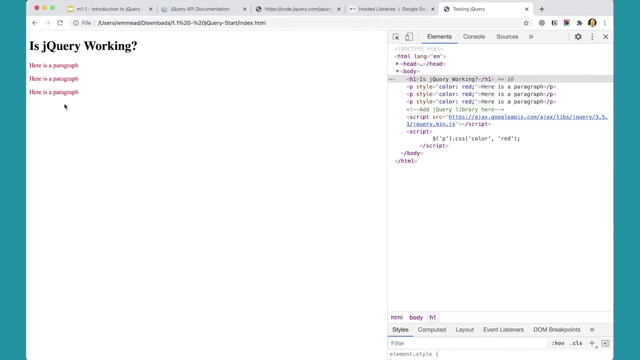 So I can just grab the paragraphs and say CSS color red. Okay, And you'll see over here, when I run this page, it's loading those paragraphs and it's turning them all red without having to do a loop, And that saves me a lot of, not a lot of extra lines, but a few extra lines of programming. 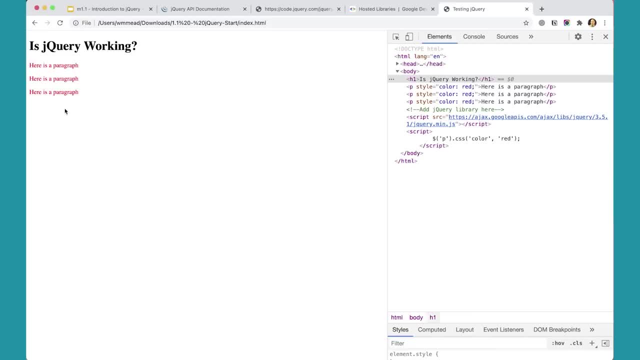 And it's one of these. this is the kind of thing that makes jQuery easier to get into for people who are new to programming. This whole thing of having to- oh, I take this array, now I've got an array. now I've. 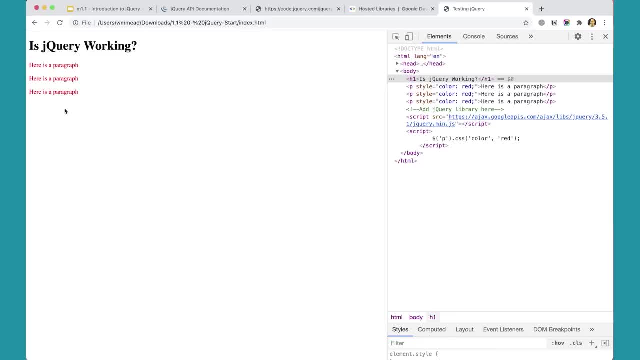 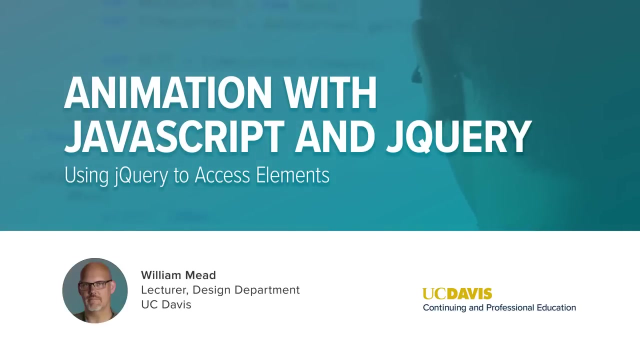 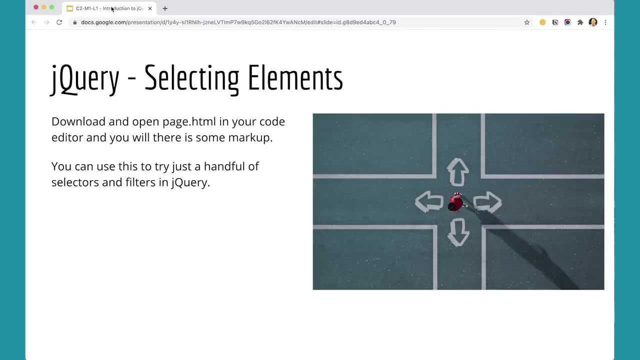 got to loop through it. It's a little bit of a pain. So jQuery kind of takes some of that pain away and that's really kind of a nice feature of jQuery. jQuery Selecting elements. Download and open the pagehtml file in your code editor that goes along with this particular. 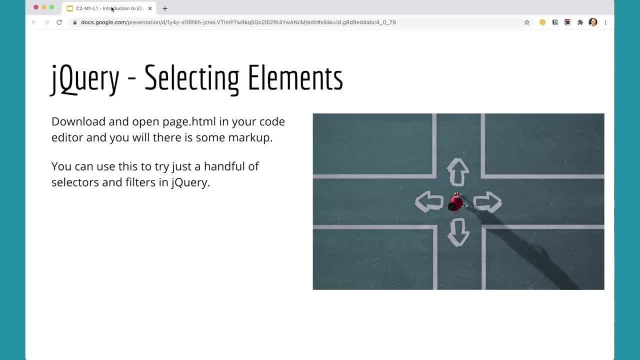 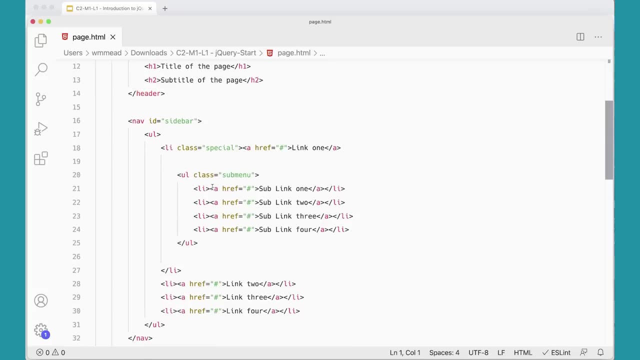 lesson And there you'll see some markup And we can use the jQueryhtml, jQuery language to select different elements in the page. If we go look at this page really quickly here, you'll see that it just has some content. It has some different markup of the header in each one and each two. some unordered lists: 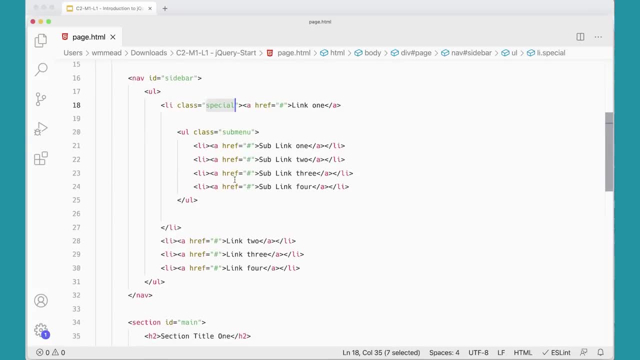 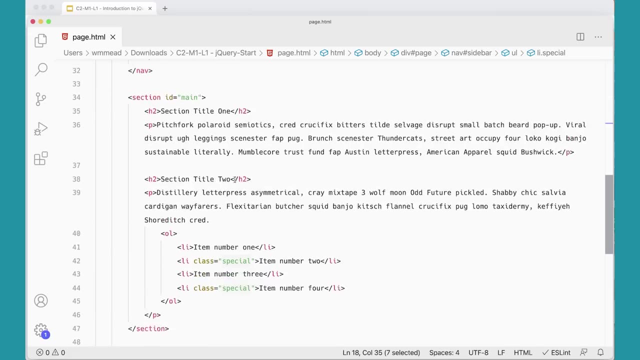 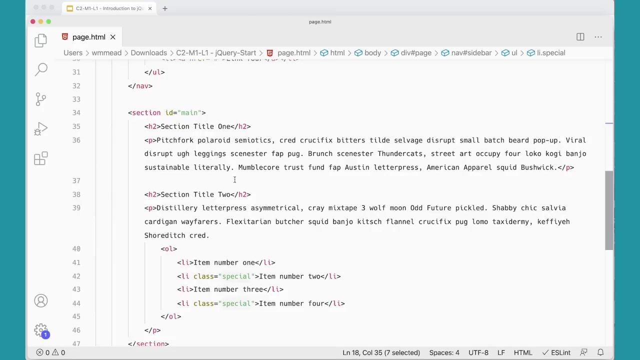 It's got some IDs and some classes and some links and some other content that we can access, And one of the beautiful things about jQuery is that you can access any element on the page with jQuery, usually in many different ways. It's the very powerful part of jQuery and you can think of it as the query part of jQuery. 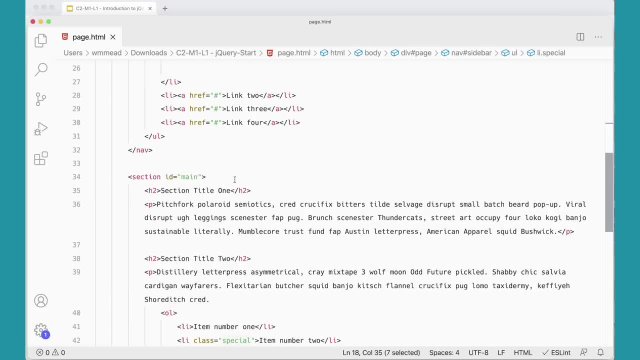 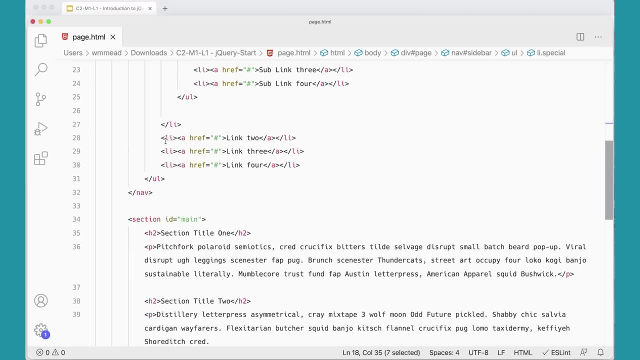 You're querying your page, you're finding elements on the page so you can do things to them or with them, or for them, And that's a very powerful thing. So we will be using jQuery to go in and access elements in this page and we'll practice that. 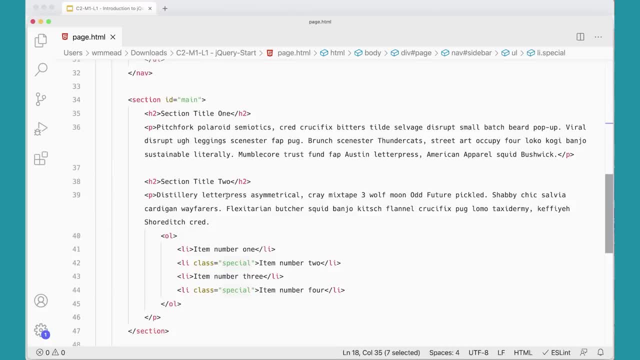 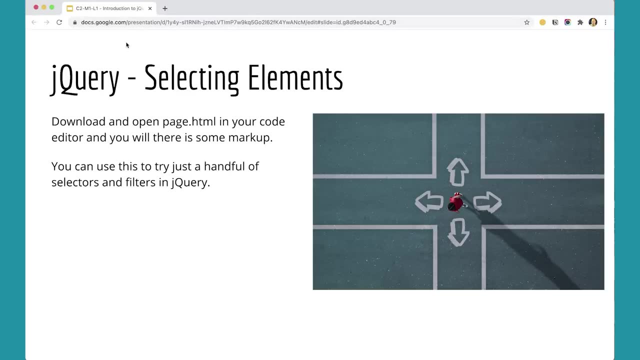 to sort of see what some of these different methods are and some of the different things we have available to us, See what they are in jQueryhtml, And that's really kind of fun and a very powerful thing to be able to do with jQuery. 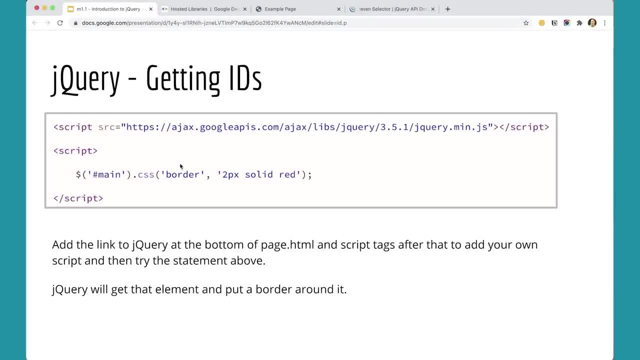 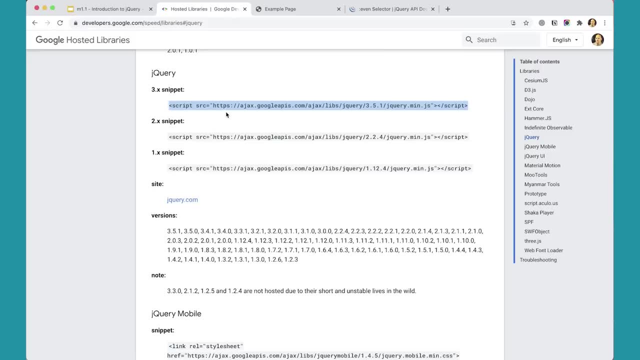 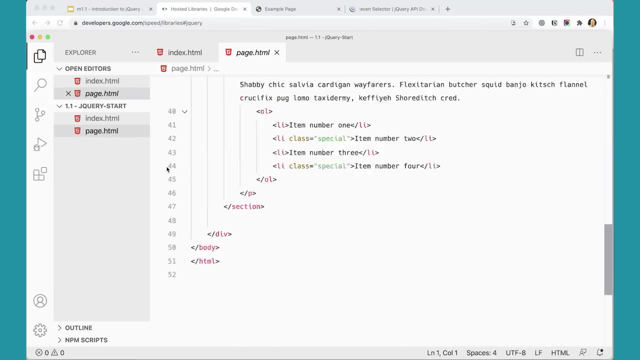 So, for example, if we were to try to do this, we could go back to our file. we're going to have to add the library again, so we need the script here. and if we come back over to our file, you'll notice at the bottom we don't have any script tags. 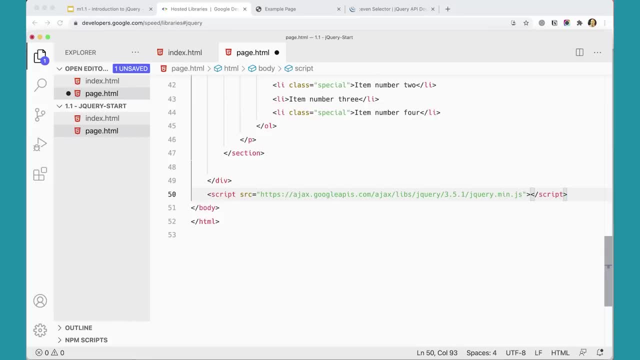 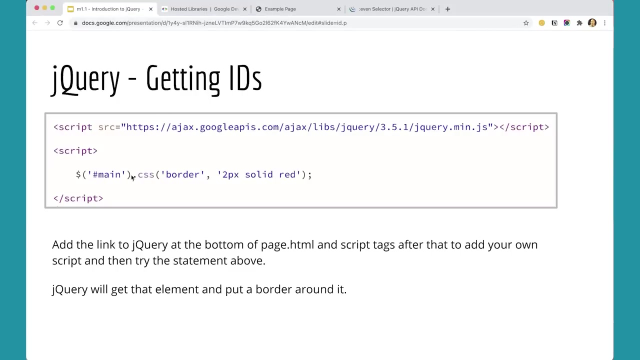 So down here, after this closing div, we need to add the jQuery library So we can use jQuery, and then we need to use a script tag which we can open and close. And now, if we wanted to do something like, for example, put a border around this main, 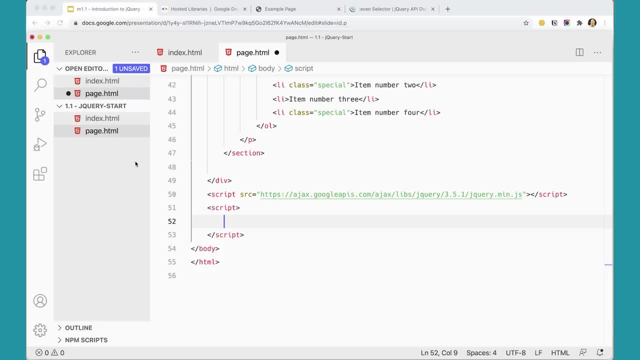 element here. we can very easily just use our jQuery object and type it. this way It'll get. There is still some syntax that you have to get used to with jQuery, But if you want to use it, you can. But if you want to use it, you can. 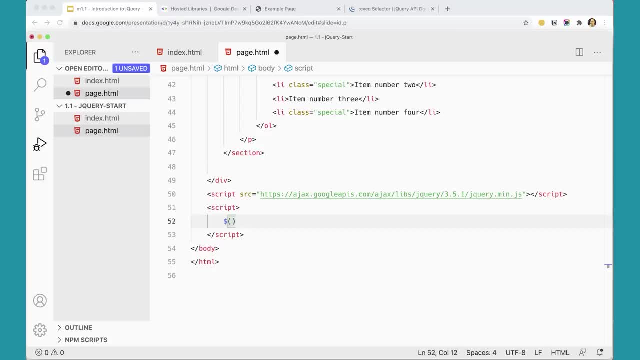 But if you want to use it you can. So I recommend typing it this way so that you can kind of get used to it. But if you do pam main and then css, the css method that we've already talked about, and we're just going to do a border here, 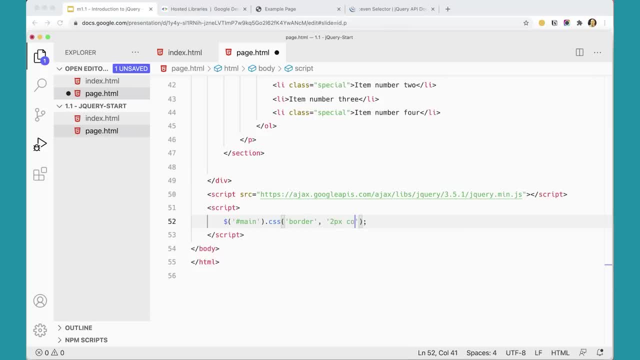 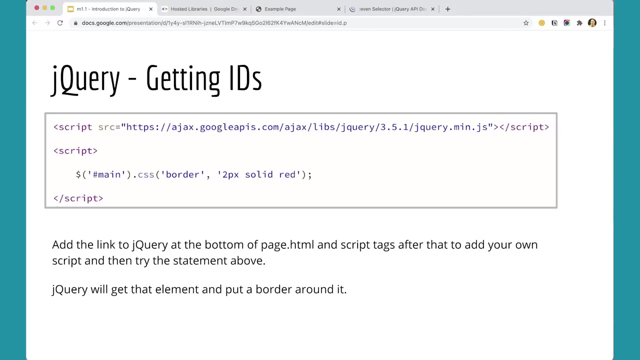 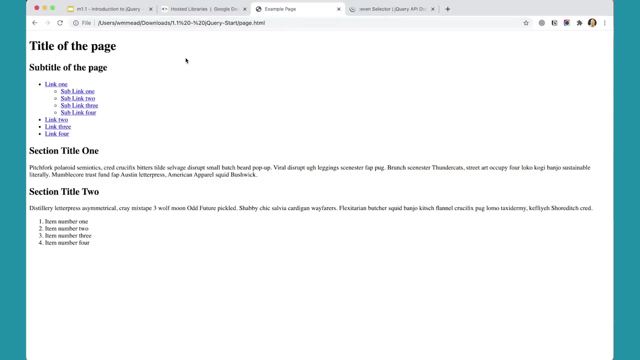 Border: 2px. color: 2px solid red. Like that I think it will work. Is that what I had over here? I think it is, Yeah, 2px solid red. So if we do that and save this document here and then come over to our example page, so 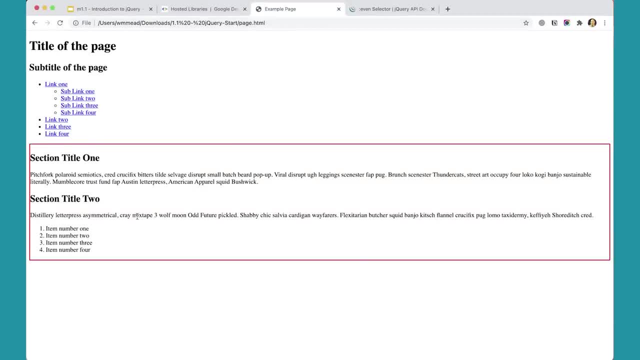 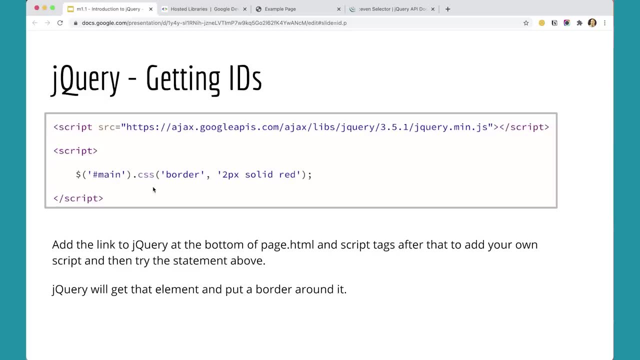 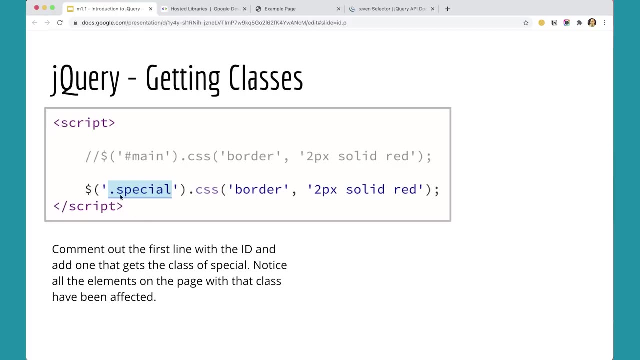 here's my page and if I refresh, you'll see I get a border around the main area of the page. so that's working. so we can access this element. we can access all kinds of elements with jQuery. so if I wanted to get the elements on the page that have the class special, so if we go back to 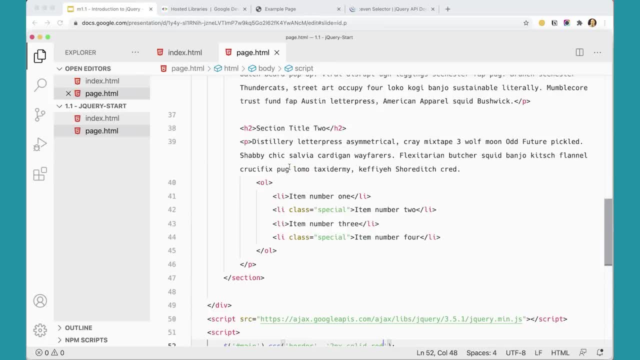 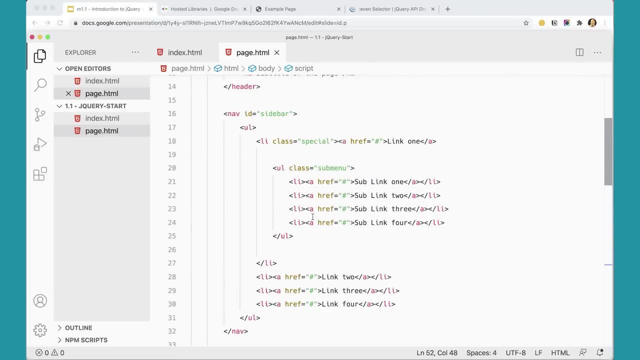 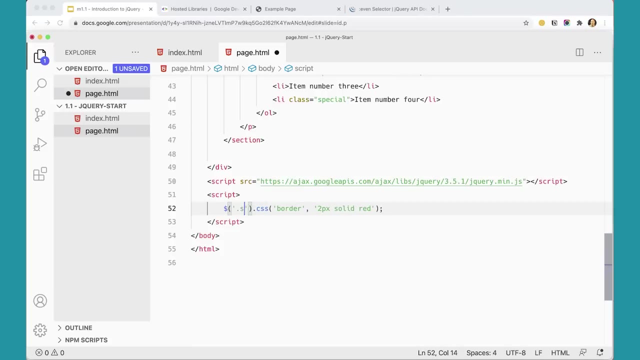 our code here we should see that we've got a class special in these two list items. we've got a class special up here on this list item, so these items should be targeted if we change this to dot special. and one of the things that's nice about jQuery is that if you just know CSS, then you know. 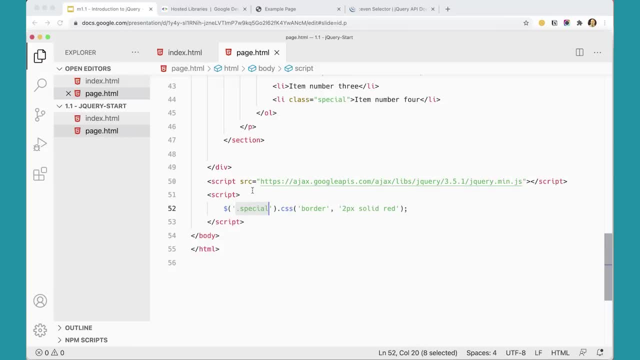 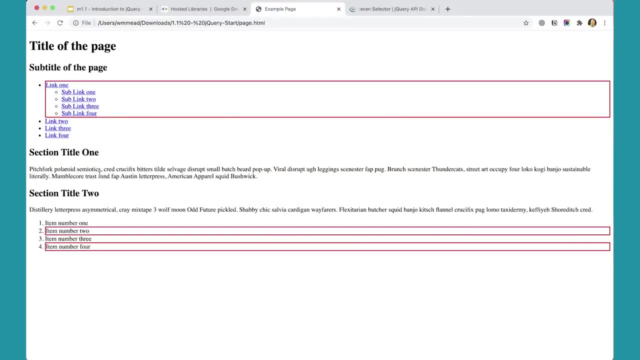 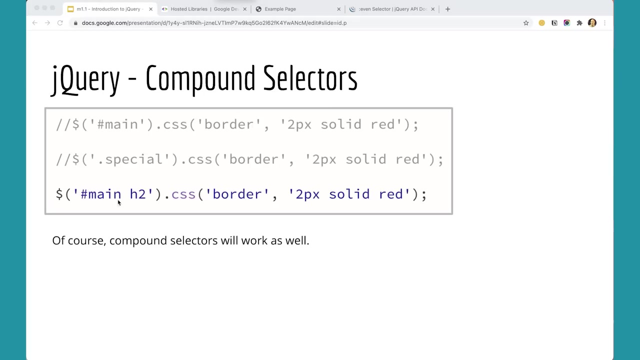 how to get these selectors. it's just using the same selectors you use in CSS, so I can come over here and try that again. you can see those elements are getting the order around them. you can also use compound selectors, so if I wanted to get specifically the h2 inside of. 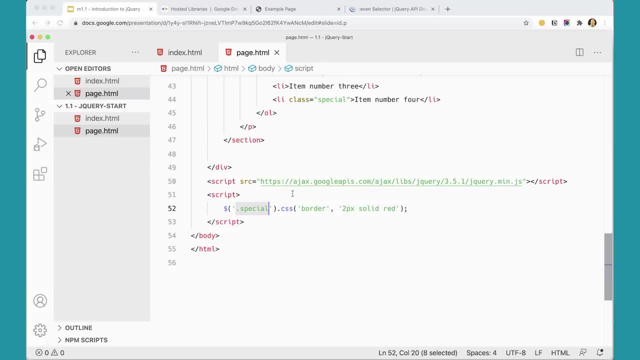 main. you can do that as well, so we can do h2 now. this may not seem so special now because we have query selector in plain JavaScript which allows us to use compound selectors like this using the CSS index. but back in the day, when jQuery was invented, you couldn't do this. 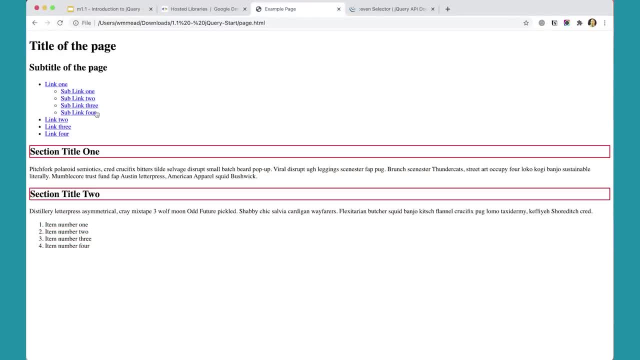 that stuff in JavaScript, and so it was a lot more complicated to be able to get to elements in the page with plain JavaScript. Now it's not so hard, but still. this is pretty neat to see that you can get to these elements really easily inside of our page and, you notice, I don't have to do any kind of looping. 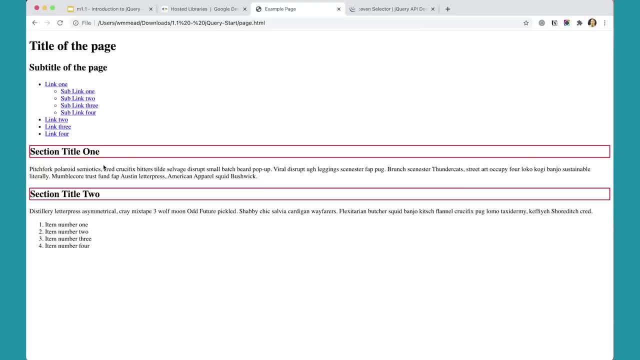 so even if I was using plain JavaScript even now, with query selector at all, I would have to have some sort of loop or for each method or something like that to go through and turn each one of these red, Whereas in jQuery I can very simply just 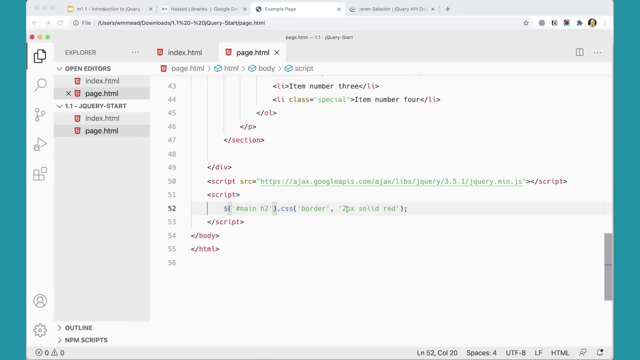 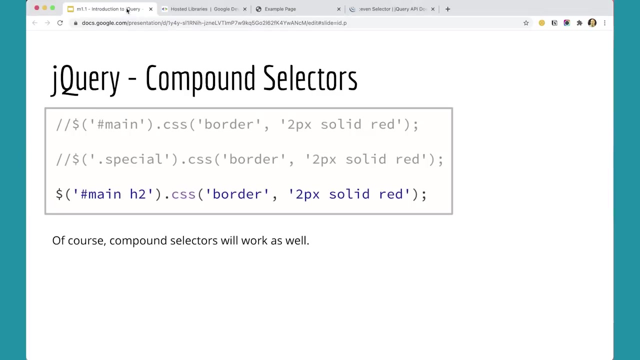 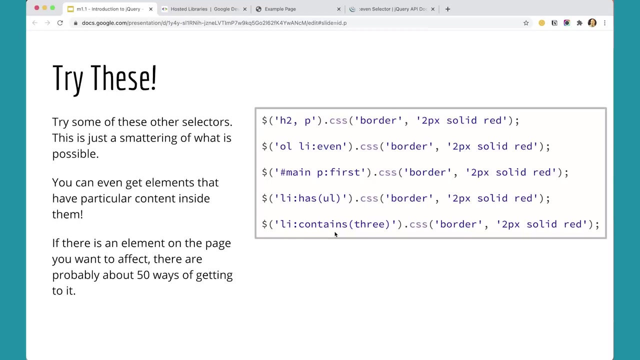 grab the group and apply the CSS to it and applies it. So this thing returns a jQuery object with these elements inside it and then we can apply that CSS to it. So that's pretty nifty. There are more that you can try. So, for example, you can try multiple selectors. like I can say I want. 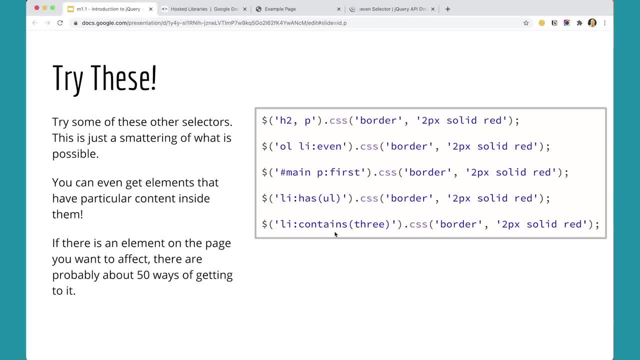 the h2 and the paragraphs. I recommend trying these out. I'm not going to make you watch me type them all. I could get the even list items, or the first paragraph, or the list item that has an unordered list inside of it, or a list item that 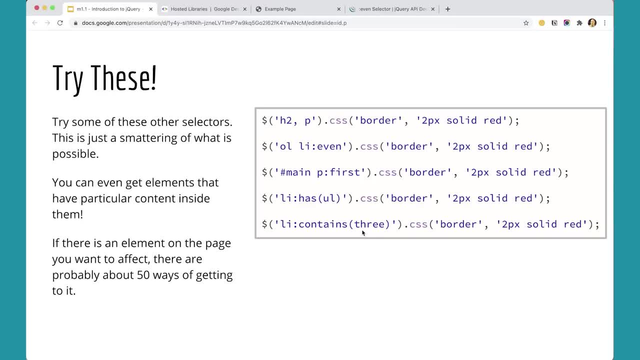 contains the word three. So there's like all of these different ways of getting content under jQuery. Now, some things to pay attention to is that jQuery does change over time, and some of these that I have on this slide was some of these that I have on this. 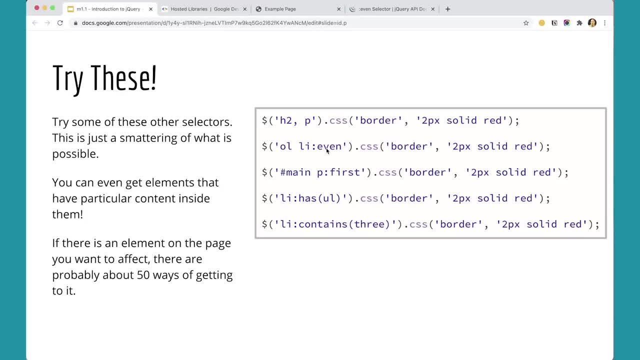 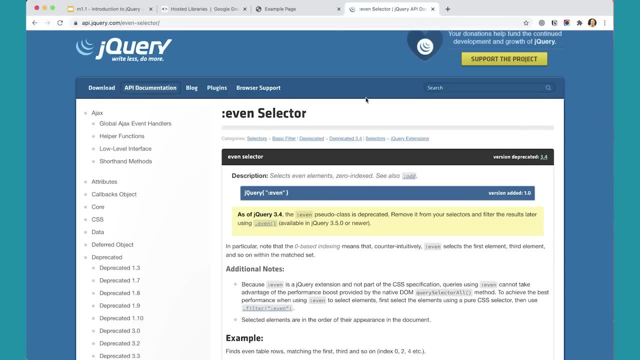 slide are are actually deprecated now. So, for example, even in first, we're not actually supposed to use anymore. If you come over to the, to the documentation, you'll see that, as of jQuery 3.4, even the even pseudo class is deprecated. but they want you to use instead is even. So let's take a look at how you would do. 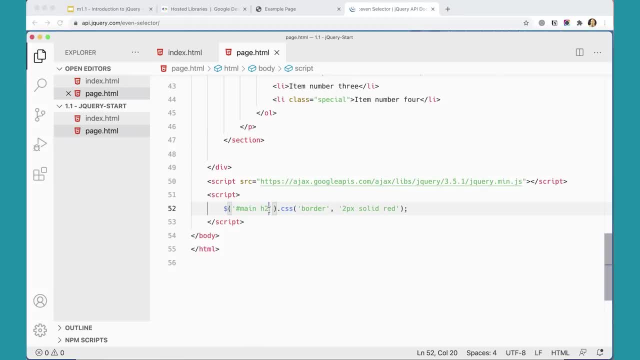 that. So over here, if I did, instead of saying li, colon, even I would do li, and then I would do even css like that. and this is called chaining in jQuery, where you chain one thing to another and so I can actually do that. 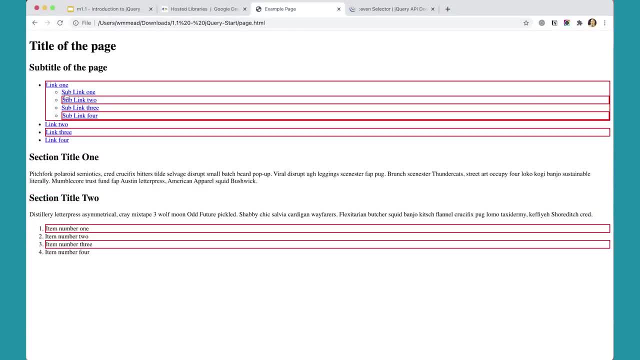 Let's come over and see what that gives us. So that should give us the even and notice it's starting counting with zero. so this is this is number zero. then, within the sublist we've got, this would be the even ones here and there and then even ones down here. 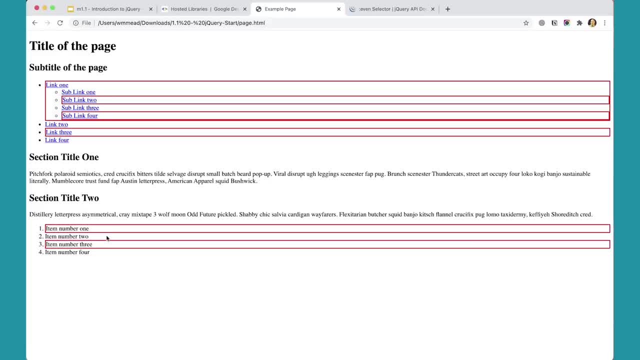 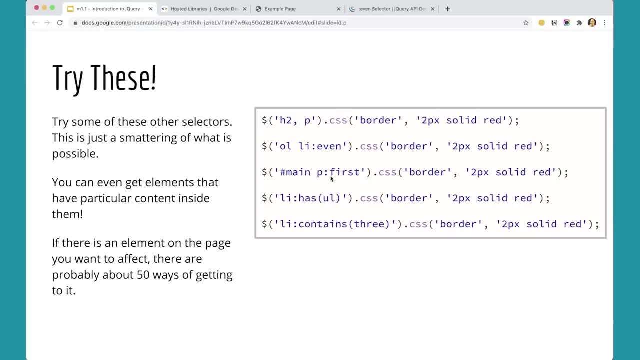 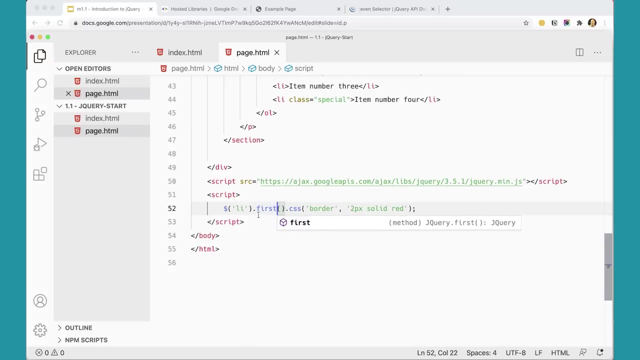 0, 1, 2, like that, so it's getting even elements. the other- the other one that is is not supported anymore- is first. So you would, instead of using first colon first, you use first, like this, and that will get the first list item in a given list. 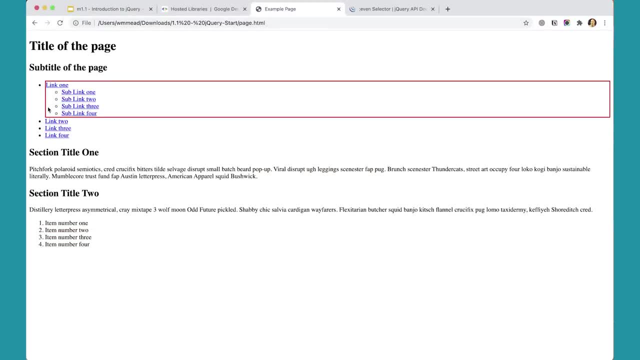 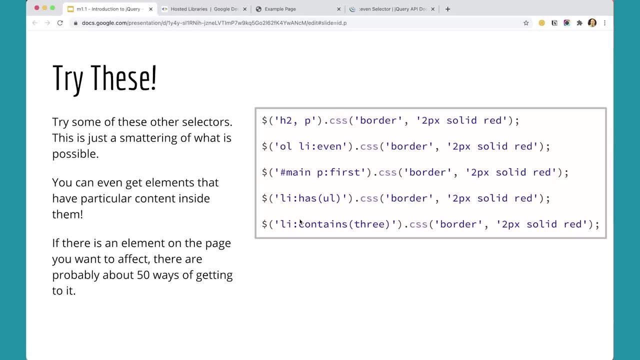 let's see what that gives us. so that gives us this first one here, okay, so, um, so there we go. uh, that's how some of these different selectors work and, um, i recommend trying some of them out. there are so many ways of getting elements on on the page with jQuery and you're not going to. 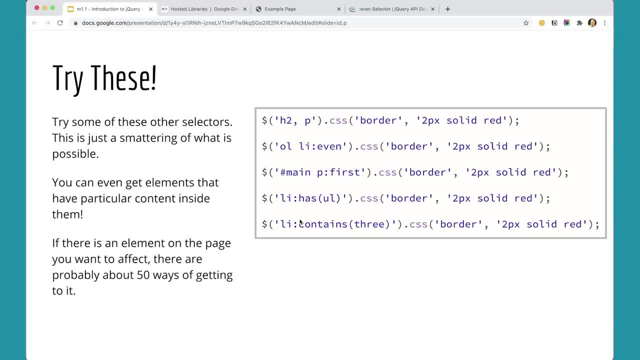 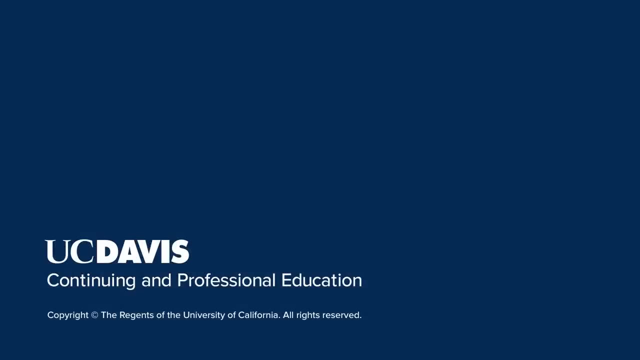 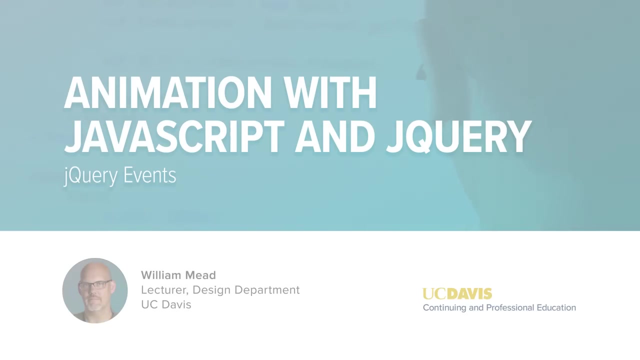 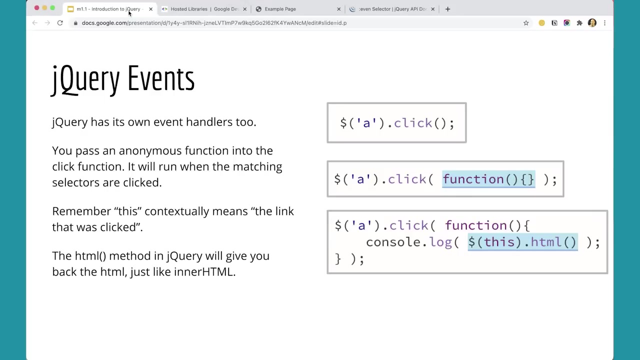 remember them all. the best thing to do is, when you have a page and you have some elements, you need to get to be creative. use the documentation for jQuery to help you find the best way of getting to that element on the page. let's look at how we can capture some events in jQuery, and jQuery has its own special syntax for. 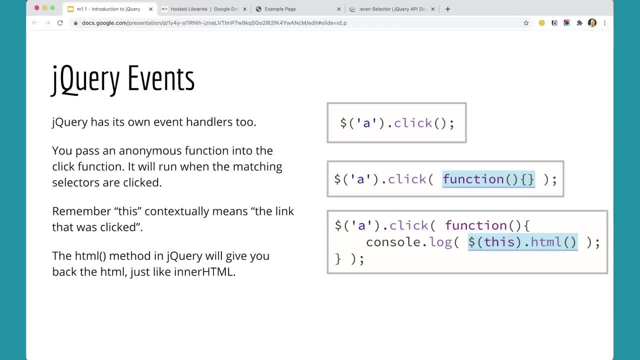 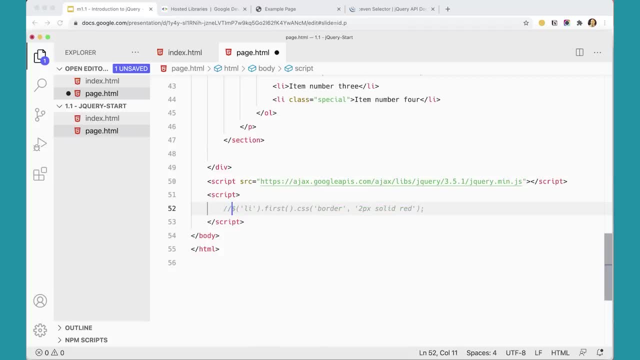 event handlers. so let's take a look at how to do that. if we come back over to our test page here, you can just comment this out or delete it just to get rid of it, but i'm going to target anchor tags on the page. so again, i'm going to type my jQuery object and in there i'm going to say a: 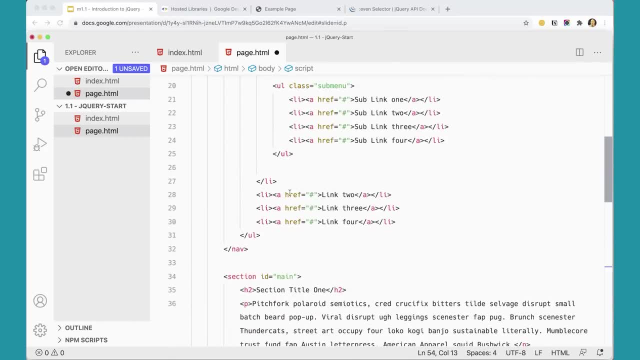 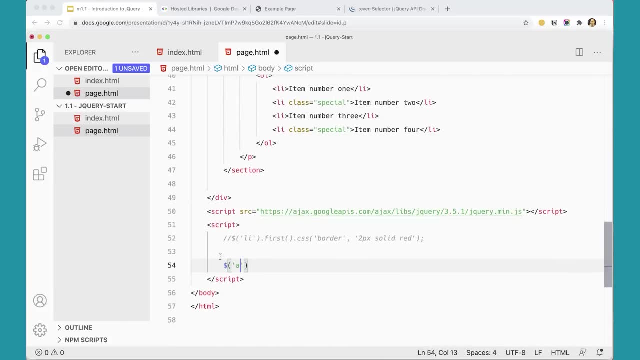 so that's going to go in and target all of these anchor tags on the page, all of those and all of these, and that's going to put that, gather all those items and return them in this nice little jQuery object here. and i'm going to add a click handler, dot click, so this click handler is going to fire when you click. 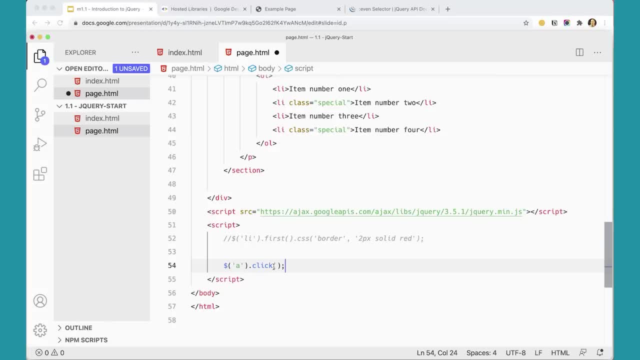 on one of, on any one of those anchor tags and what i'm going to pass in. make sure you type it this way, so you're typing from the outside in. i'm going to type, i'm going to add in here a function, function, oops, like so, with curly braces, parentheses and curly braces. so this is an. 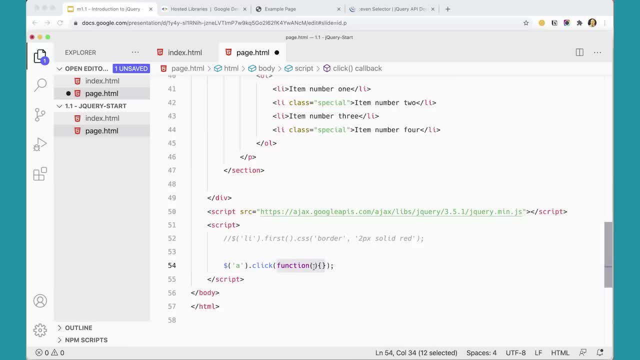 anonymous function. this is a function that's just going to run when we, when this click handler happens and in here i'm just going to put consolelog, i'm going to put in here i'm going to put this dot in html and that should put in the console the html of the link that i clicked, because it's going to. 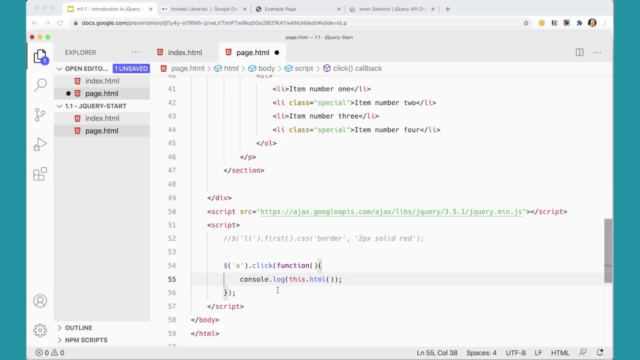 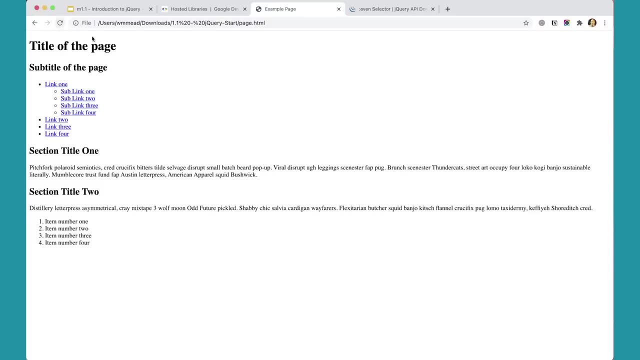 put this in all of the links. i can only click one link at a time, so let's see what this does if i come back to my example page here and refresh it and then turn on my inspector here and turn on the console if i click a link. 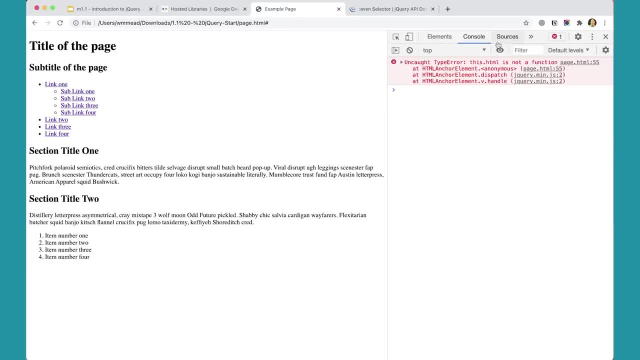 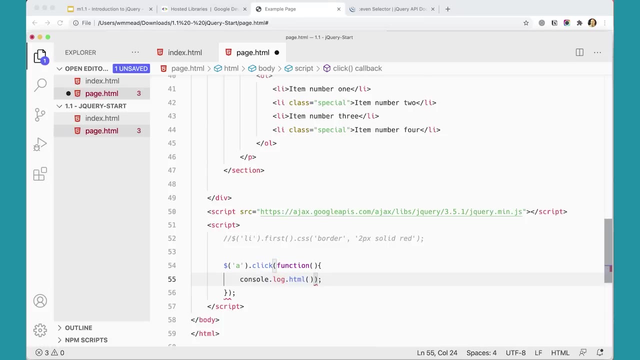 oops, thishtml is not a function. i must have done that wrong. i know what i did. come back over to visual studio code. this needs to be. i need to use my jquery object, so i'm having all sorts of trouble here. dollar sign, parenthesis, this all right. so i'm using jquery to get this, and now i'm going to write this command to this: l häufig privateóg. 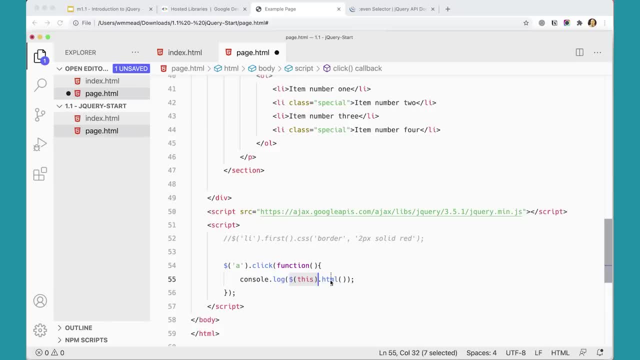 jquery to get this, and now i'm going to read what's there and this is going to get 99.6 billionな. And then I'm using a jQuery method called HTML here that's going to return the HTML. Let's see if that works. 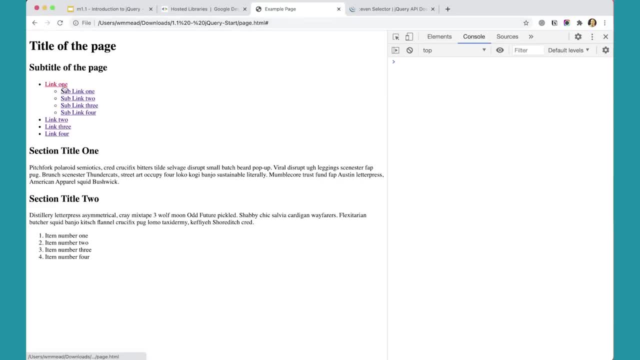 Test that again. Click a link and I'm getting link 1.. Or if I click sublink 1, I get sublink 1.. Or if I click link 2, I get link 2.. Link 4, I get link 4.. 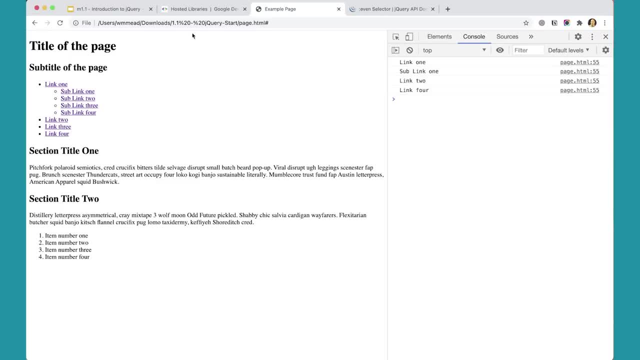 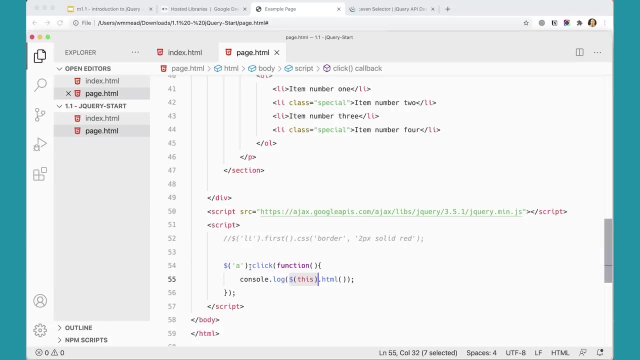 So what's going on here is that the click handler- and this is again in plain JavaScript- we would have to use some sort of loop to apply the click handler to all of the anchor tags, But here I can just grab all of them, return them in this jQuery object. 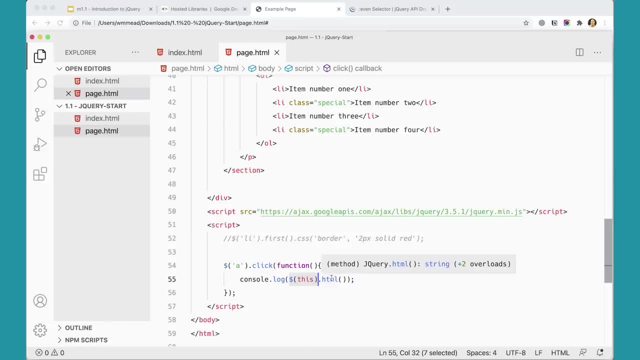 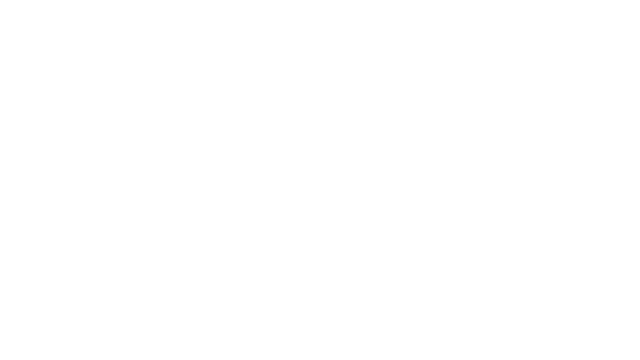 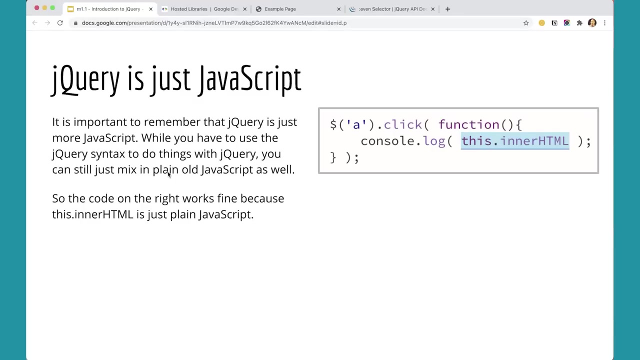 and then I can use this method here- consolelog- to tell me what is inside of these anchors, Anchor tags, each time you click on one. So that's pretty nifty. The next thing to keep in mind is that jQuery really is just plain JavaScript. 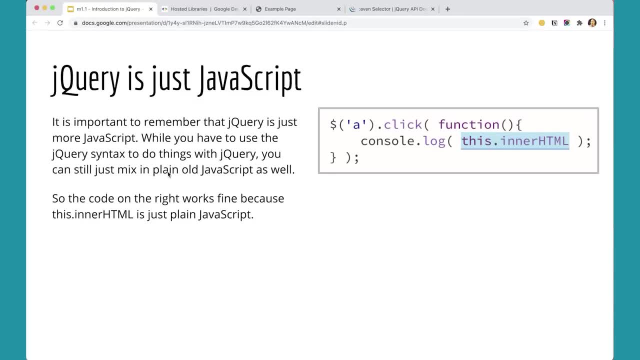 It isn't a separate thing from JavaScript. It isn't a separate language, It is just JavaScript, And you can mix in regular JavaScript with jQuery. That's why I made the mistake I made a few minutes ago. I was trying to do a combination of the both. 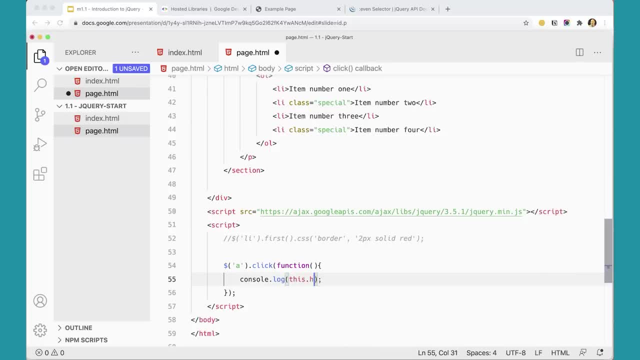 But I can just do thisinnerHTML And that should work exactly the same way, except that this is using plain JavaScript here instead of jQuery to do the same thing. So if I come back and test this, link 1 gets me link 1.. 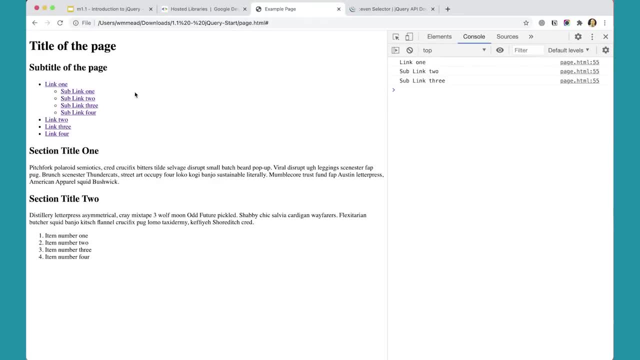 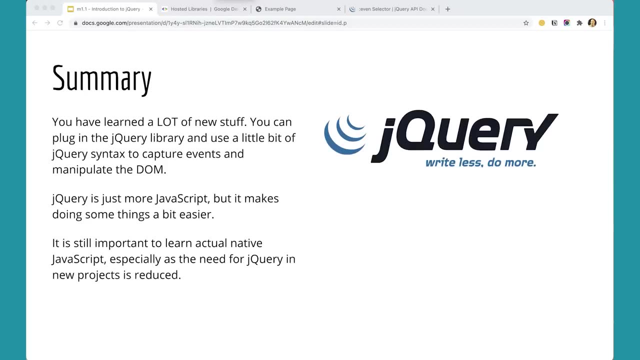 Sublink 2.. Sublink 3, and et cetera. In summary, you've learned a lot of new stuff. You can plug in the jQuery library, either by downloading the library and putting it in your files, or you can use the CDN. 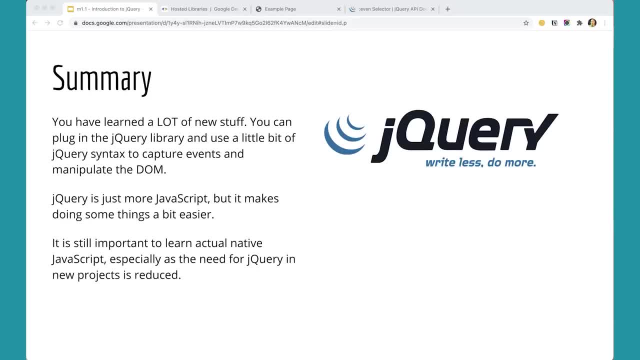 You can use jQuery to capture events and to affect elements in the DOM. There's a lot more to learn, but this is a really good introduction to what jQuery does. It's just more JavaScript, but it makes doing some things a little bit easier. 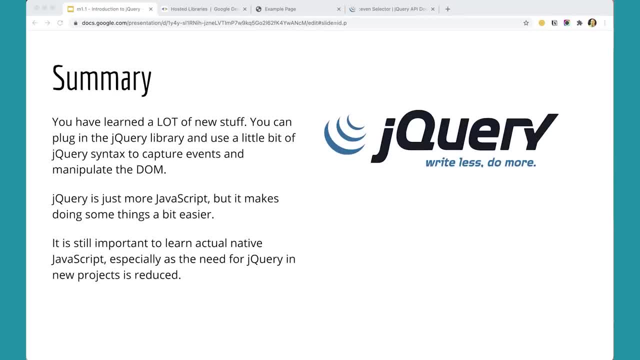 And it's still important to learn actual, native, regular, plain vanilla JavaScript, especially as the need for jQuery and new projects is reduced. But if you get a job and you're working on a project, it's very likely that you'll be working with legacy code and you'll encounter jQuery. 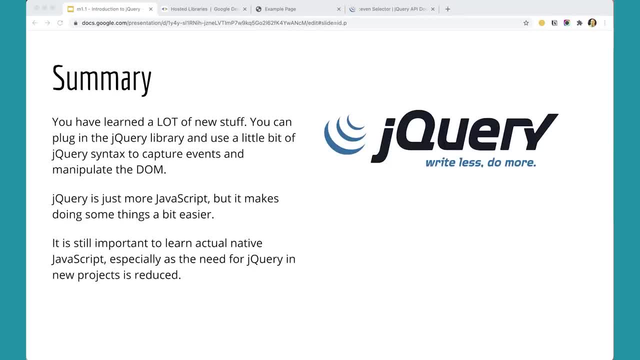 Or if you're looking around on the internet, you're very likely to come up with solutions that are jQuery-specific. So it's because it's been such a popular library. it's going to be around for a long, long time And it's still important to learn how to work with it. 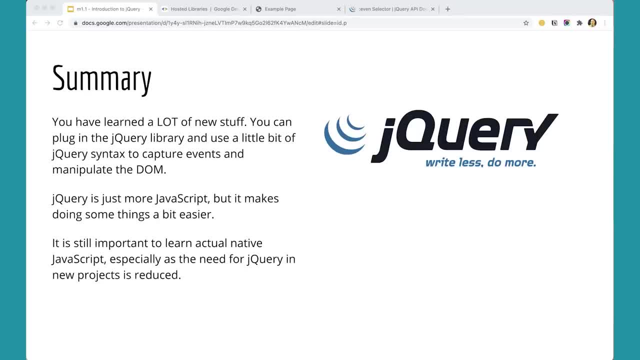 And learning how to work with jQuery will help you learn how to work with JavaScript, So it's a two-way street And I hope you have fun as we go forward with this course and learn a lot about jQuery and how to use it in different projects. 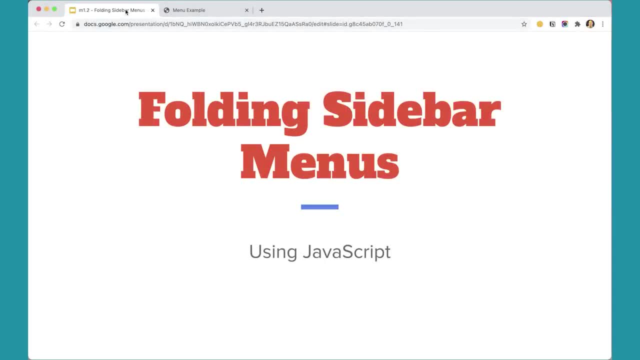 Folding sidebar menus using JavaScript. You've already learned a little bit of jQuery, But before we dive more into jQuery, we're going to do this project using plain JavaScript And then we'll do the exact same project using jQuery, And we're going to do this with a few different projects, so you can see the difference between jQuery and JavaScript. 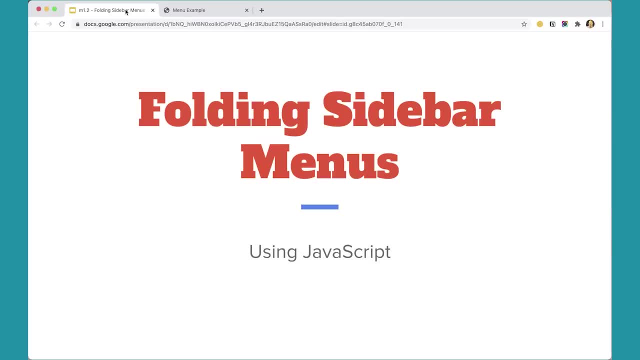 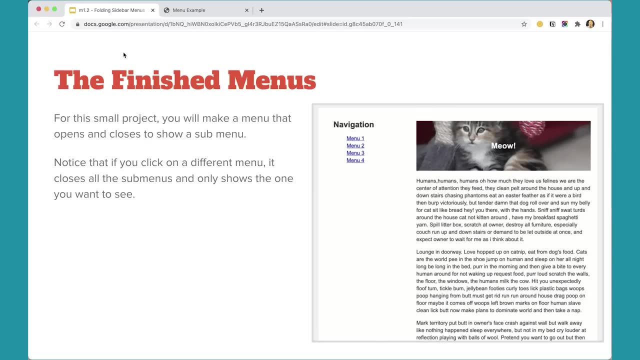 and how they work together and some of the differences between the two In this project. we're going to have just a simple page And on the side of the page we have a menu And when you click the menu item it folds down and shows the submenu. 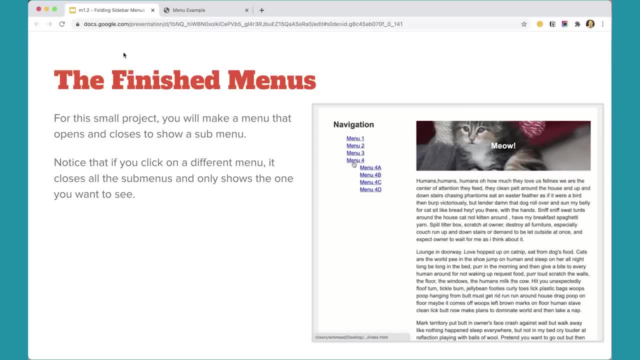 And when you click a submenu, that's well, one is already open. it will close the other one, So that will limit the number of options your user has to see, And sometimes that can be really helpful for users in terms of cognitive load. 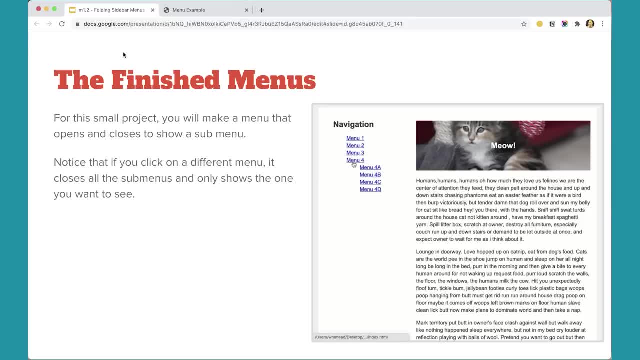 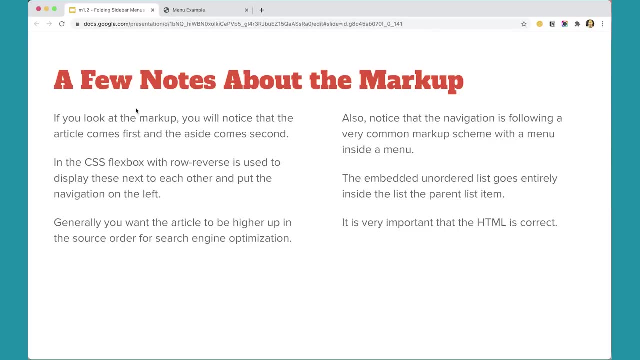 You only want them to see a certain number of options at once. So we'll look at how to build this in plain JavaScript first, And then we'll do the exact same project using jQuery. Just a few notes about the markup. If you look at the markup, you'll notice that the article comes first and the aside comes second. 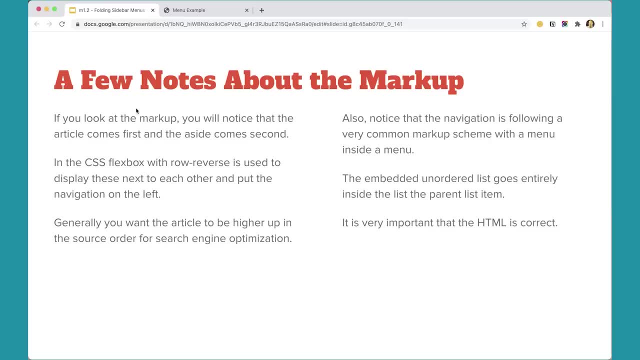 This is often important for search engine optimization. We want the important content further up the page. We'll use CSS Flexbox with row reverse to display these next to each other, but put the navigation on the left. Generally We want that first article, the article higher up on the page. 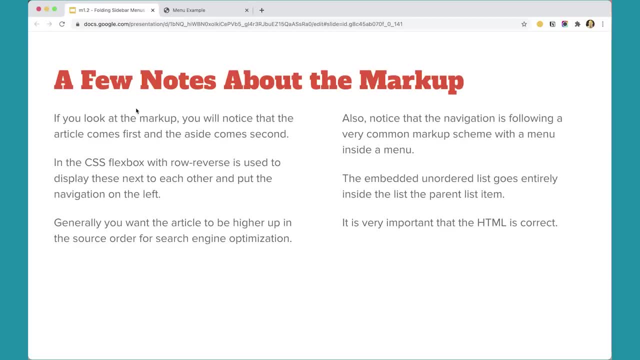 Also notice that navigation is the navigation is following a very common markup scheme with the menu. inside of the menu, This embedded unordered list goes entirely inside the list item for the parent And this is important to get in HTML. So let's take a look at this really quickly. 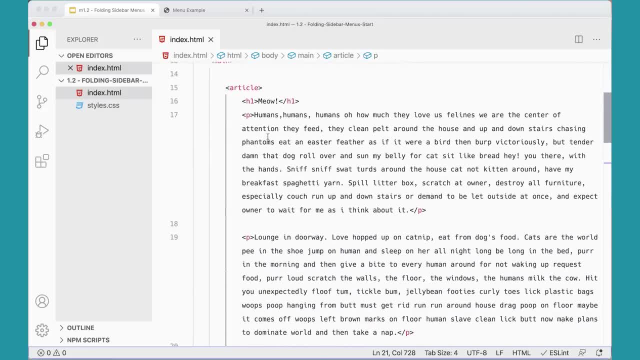 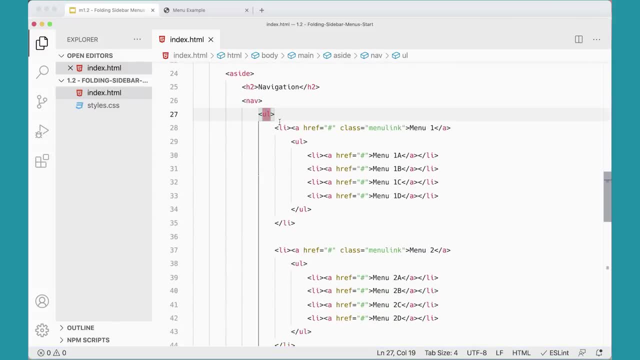 So over here I have my page open and you can see the article comes first right after my main section opens there And then the navigation is an unordered list with list items. but notice, this list item is entirely enclosed in the parent list item. 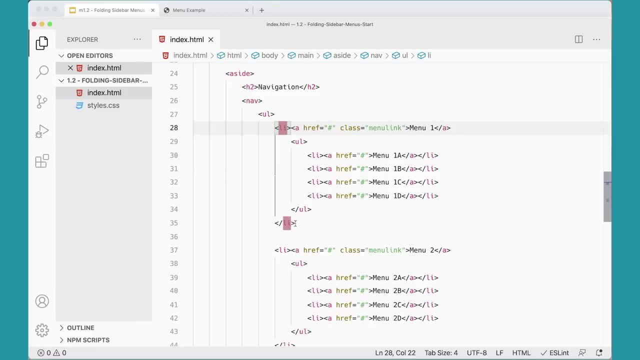 This is really important to get right and a lot of web developers get it wrong. The only items you're allowed to have as children of an ordered or unordered list are list items, So this unordered list needs to be entirely enclosed in this parent list item. 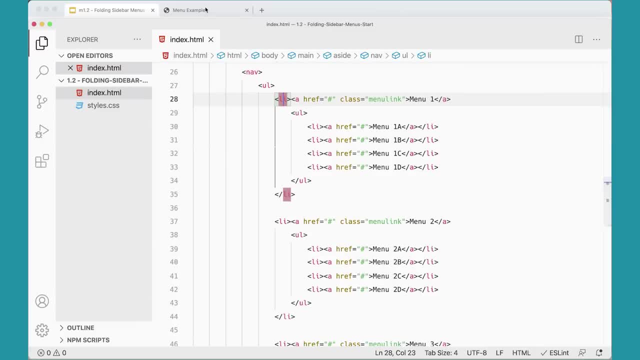 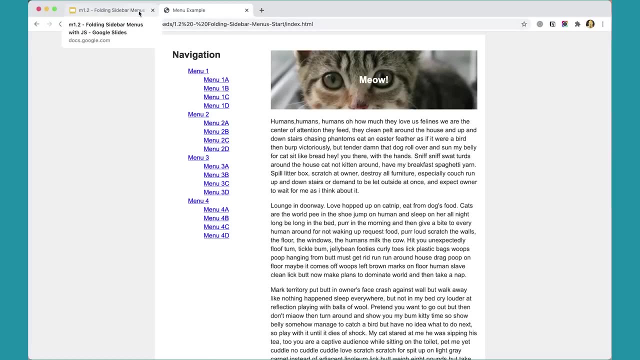 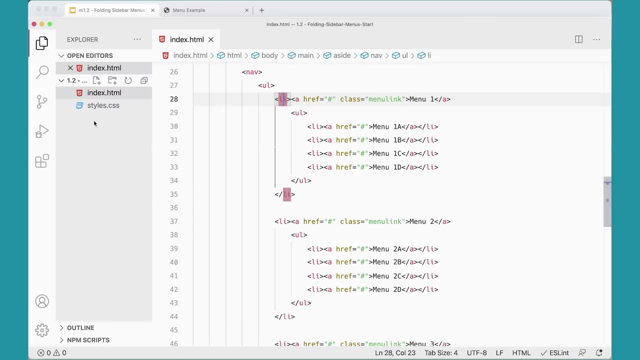 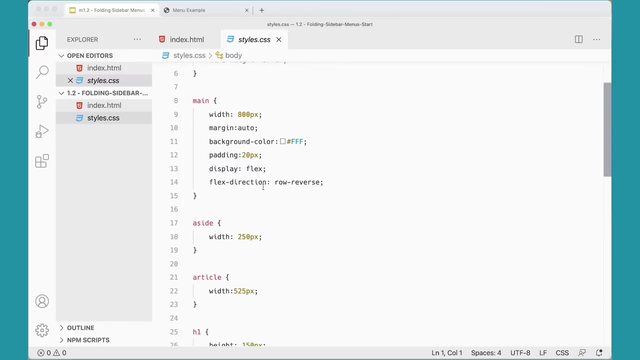 And these are the items that will show On the page. So over here, currently without any JavaScript, These items are just showing. Okay, So that kind of gets us started and we're using just a little bit of CSS here, as demonstrated here on the styles to make to display flex for this main element. but 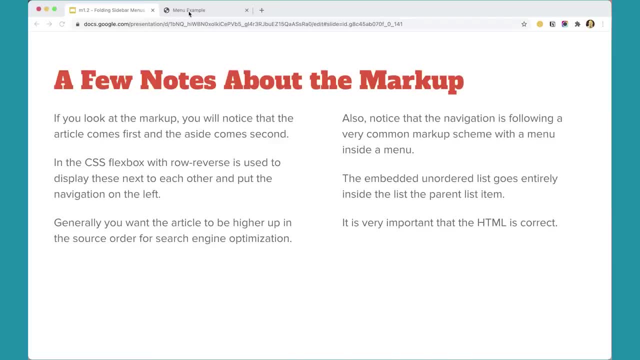 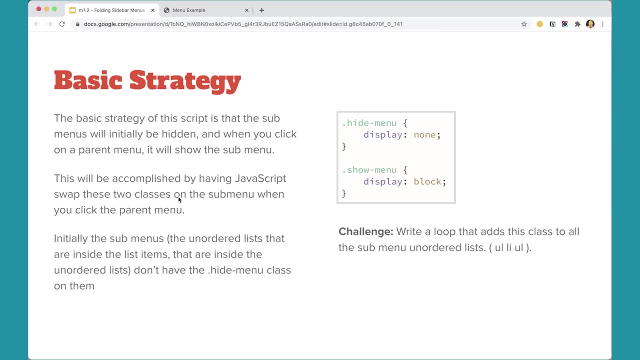 use flex direction row reverse- to get the navigation on the left And the main line content on the right. Okay, great. Now, with all that in place, let's get started with making this project work. The basic strategy of the script is that the submenu will be: 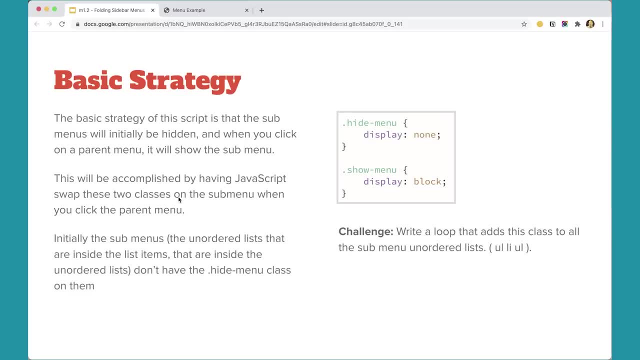 initially hidden and then, when you click on a parent menu, it will show the submenu. This will be accomplished by having JavaScript. swap these two classes on the submenu. when you click on the parent menu, Initially the submenus, the unordered lists that are: 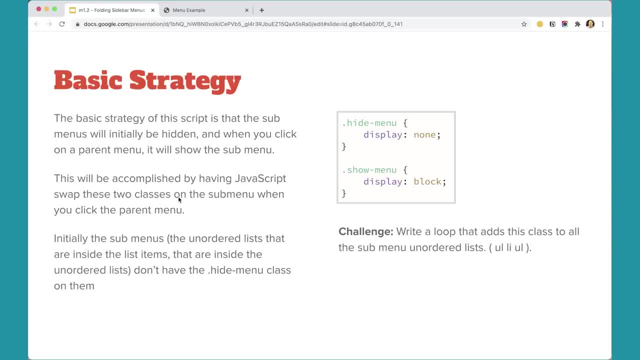 inside the list. items that are inside the unordered lists don't have the hide menu class on them, So our first challenge is to write a loop that adds this class to all the submenus in the unordered list, And you'll see over here in the style that these two 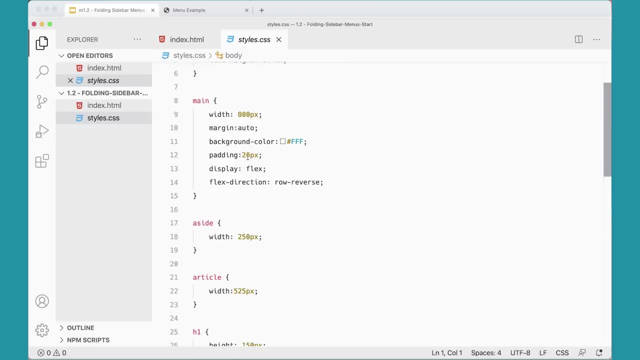 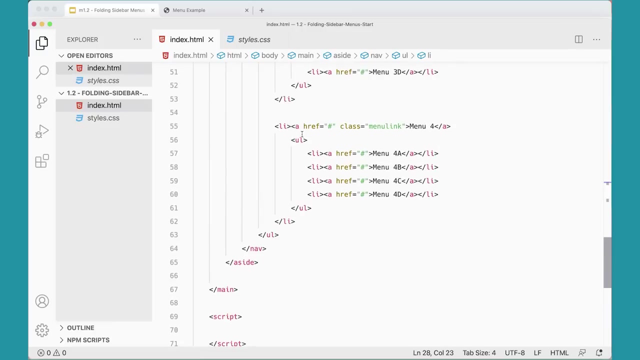 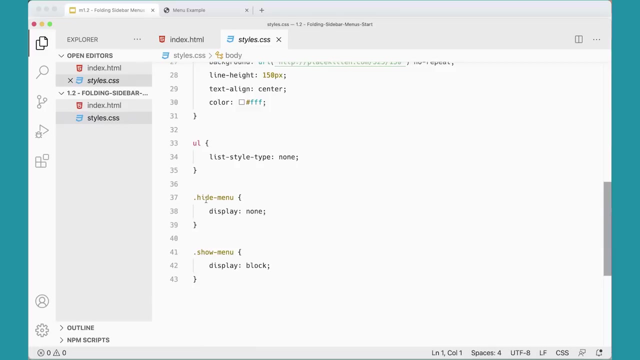 styles are already here: Hide menu Display none And show menu display block. So your first challenge is to write a little script Down here. we've got script tags. See if you can write a script that goes in and applies that submenu to that hide menu class. We want to apply that to all of these unordered lists. 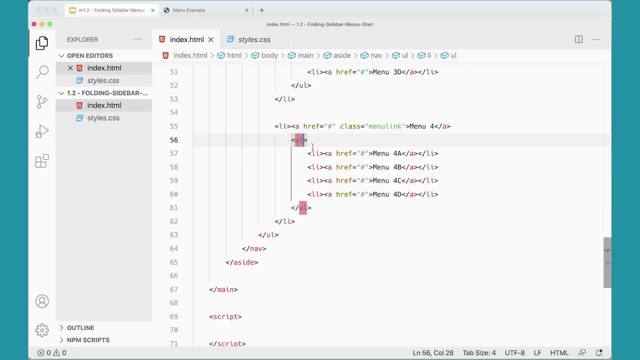 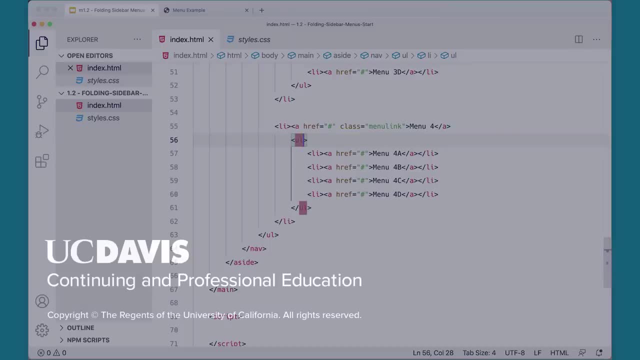 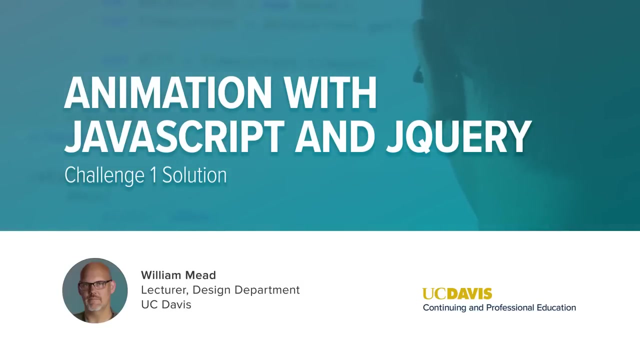 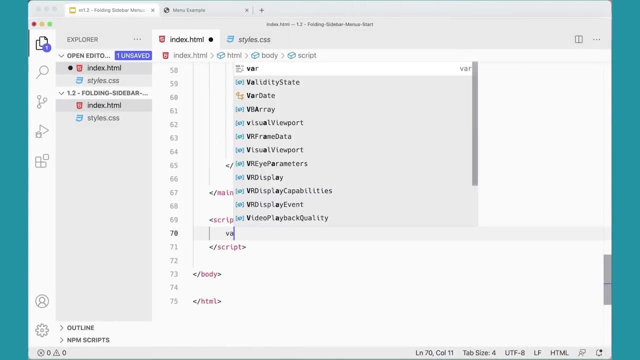 so they have class hide menu on them. See if you can do that. In the next video we'll see how I do that. Were you successful? Were you able to do it, Let's do it together Down here I'm just going to make a variable var submenus. 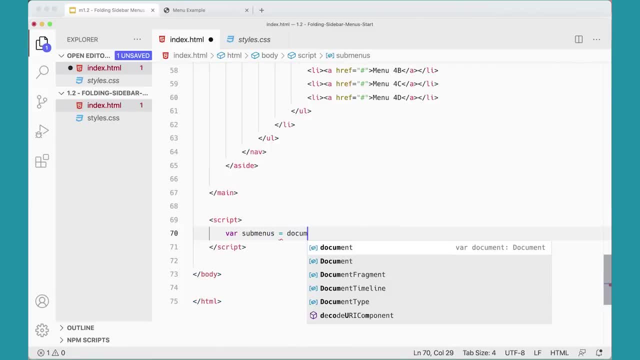 I'm going to assign that to Document dagegen dot sew query selector Selector Desk haunted where I select your all And what I want to get are the UL L-I-U-L. Whoops, there we go. 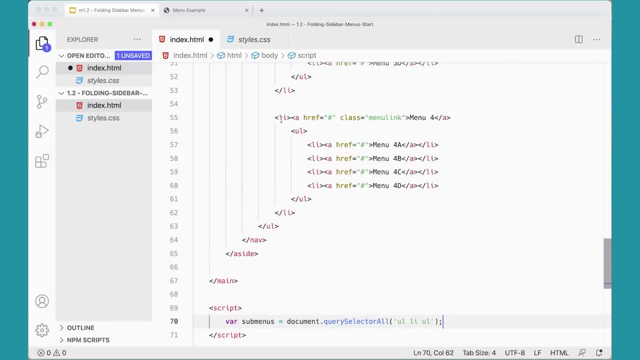 Because these, what I want are these unordered lists that are inside the list items that are inside the parent unordered list. So that's what I want to get here. So I'm gonna get these, all of these, and put them in here, And then I just need a loop for. 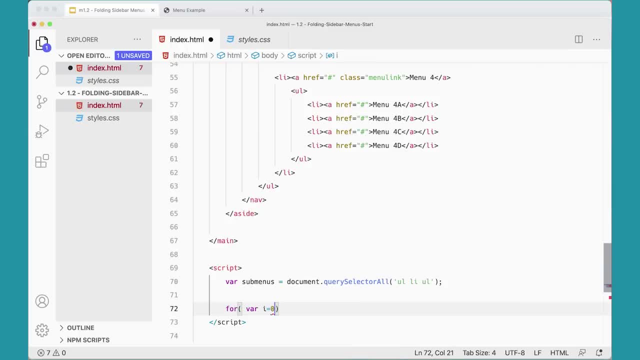 var i equals zero, while i is less than submenuslength pi plus plus curly brace. I put these extra spaces in here. They're probably not necessary, but to me it makes it a little bit easier to see this and read what's going on here. 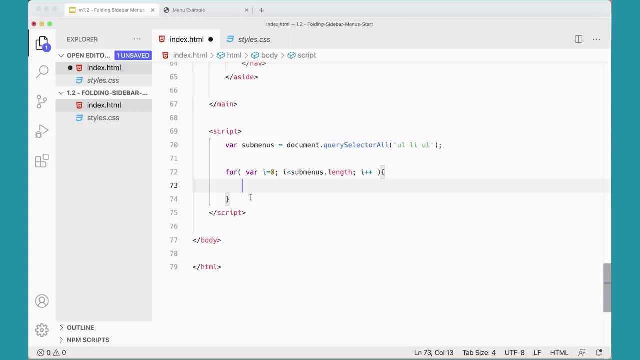 But this should be review for you, Hopefully at this point. And okay. so now here, what we need to do is we need to put that submenu on each of these. So I'm gonna say submenus dot square bracket i, So each one of these. 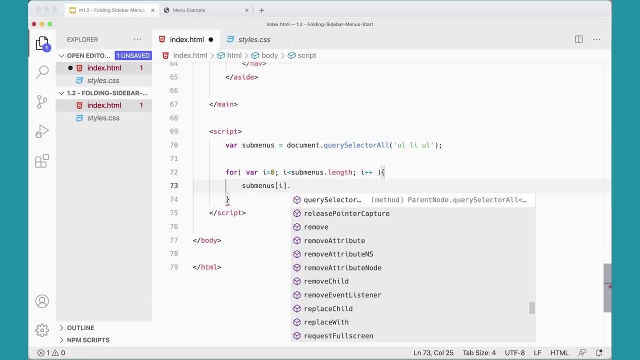 I'm gonna go through each one of these and then do class: name equals i-menu And you can have that right Over here. it's i-menu, i-menu, display-menu, And that should go through and put that class on all of those elements. 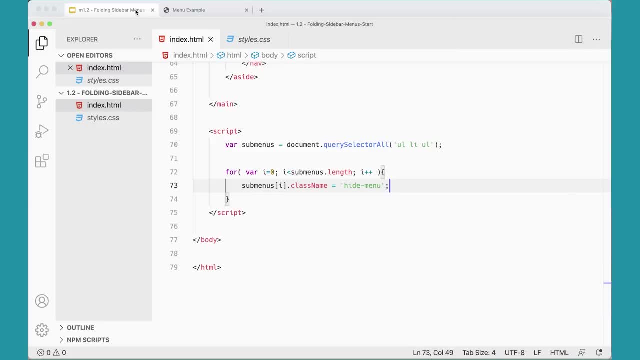 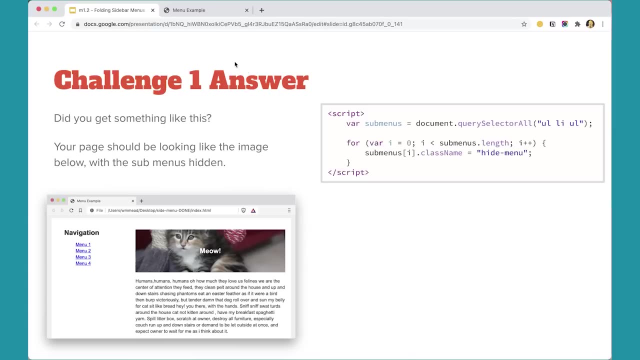 Let's see if I did that right Over here. I'll go check my document here And this is exactly what I did: class name: i-menu. So let's see if that actually works. We saved that. come over here and refresh the page. 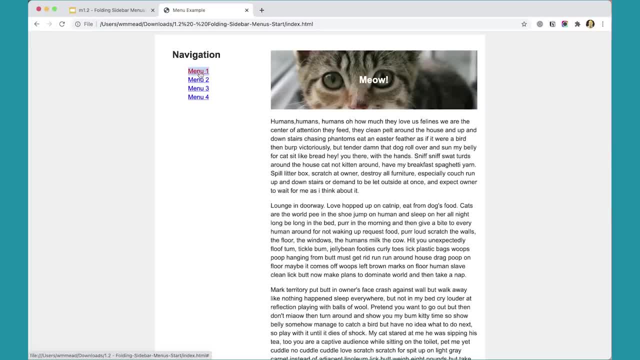 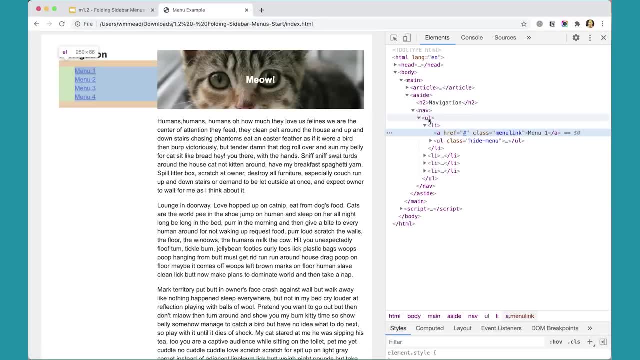 And look at that. all those menus are hidden. They're set to do. That's the display-menu I could do inspect And you can come in here and see: click on this menu here or one of these menus you can see. 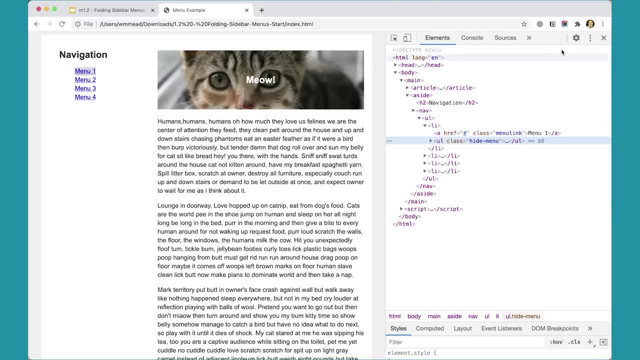 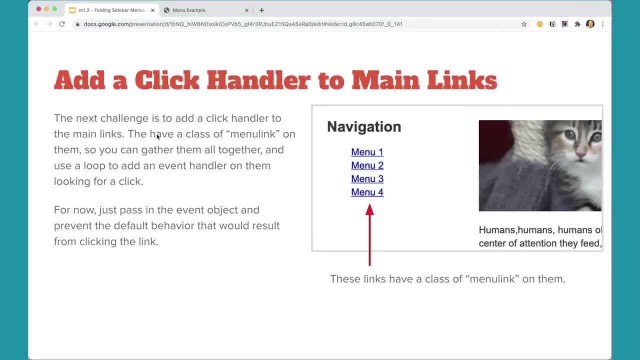 it's got hide menu on it. It's got that class on there, So that's working great. Your next challenge is to add a click handler to the main links. These links here have a class on them, A menu link, And so we want to gather those. 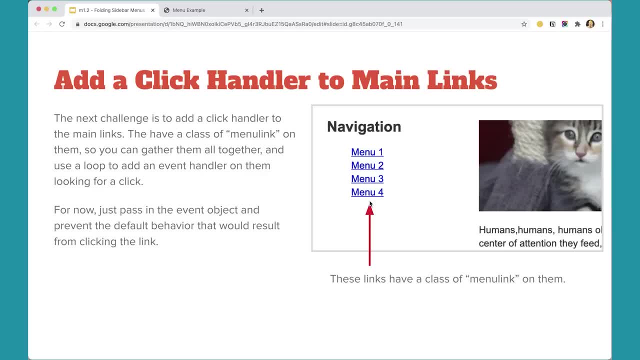 And when you click on them, we want something to happen. So we're going to need an event handler for that. For now, just pass the event object and prevent the default behavior that would result from clicking the link, But see if you can do that on your own. 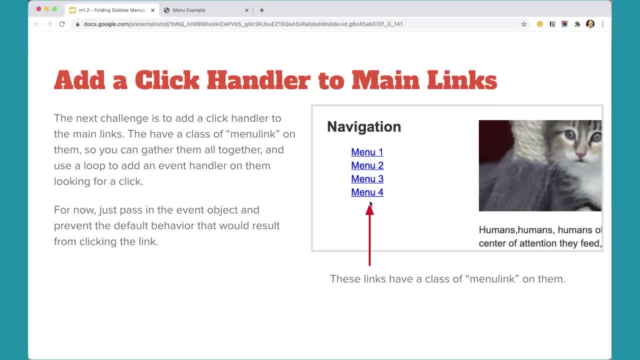 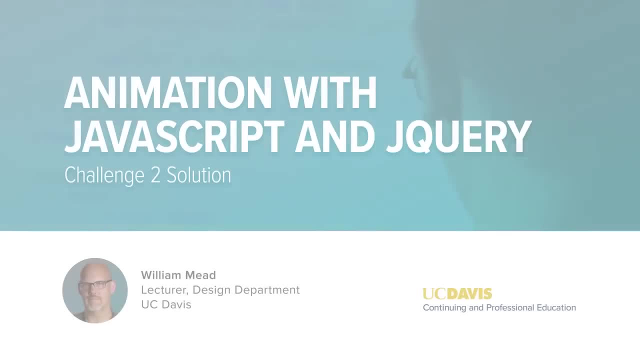 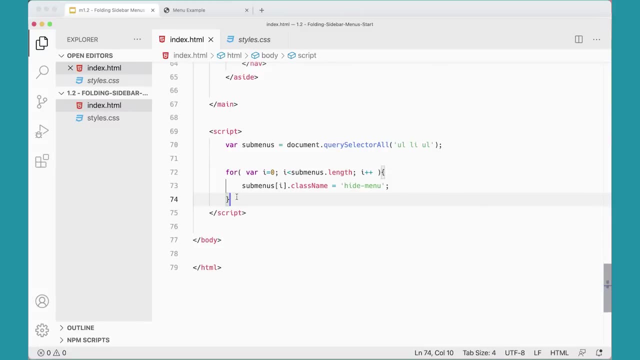 without looking at my solution, But we'll do it together in the next video. Let's do this together. So first we need a variable: var menuLinks, equals documentquerySelector, querySelector all. And what do we want to get? We want to get these links here. 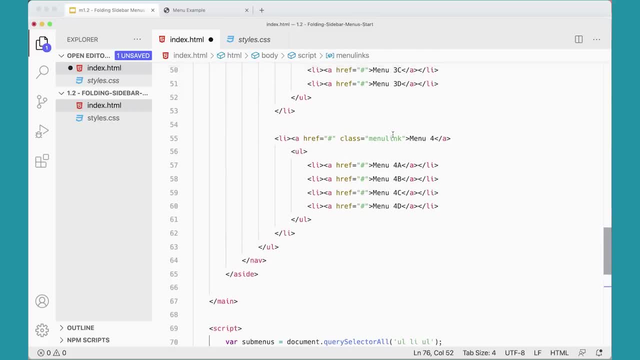 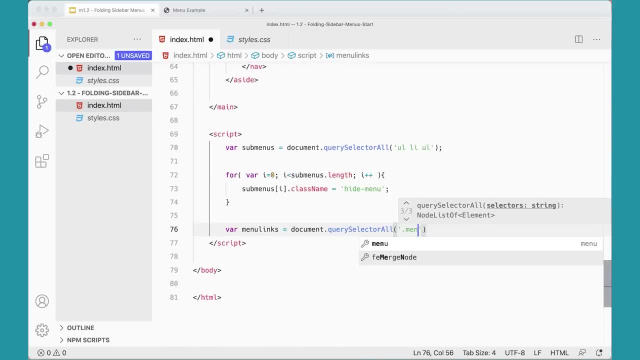 We want those. So I'm going to come up here and I'm going to do menuLink So that will get those and put them in there. And then we need a loop. We need to do a loop here, So we need a for var i equals 0.. 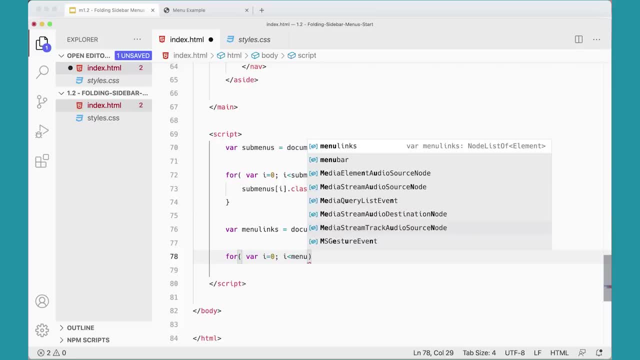 i is less than menuLinkslength i++. Hopefully you're getting used to writing loops now And then in here we're going to put an event listener on each one of these. So menuLinks square bracket. i dot addEventListener. 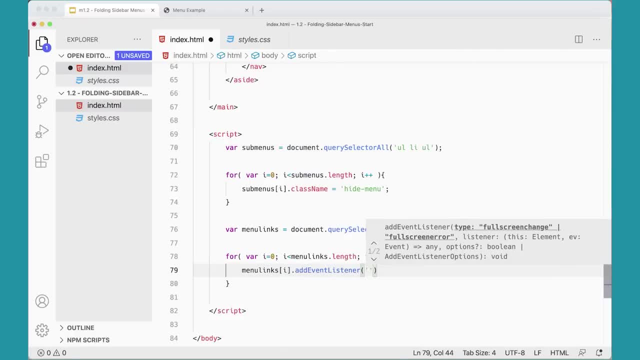 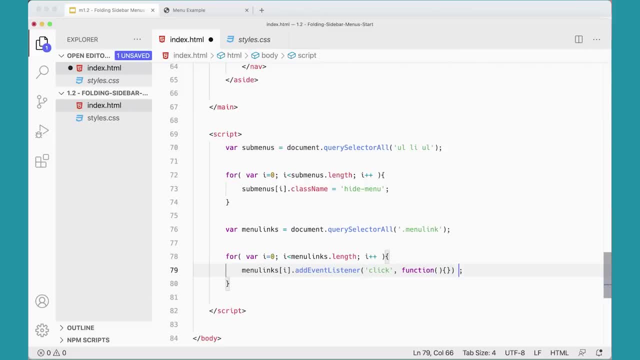 Not run an event. We're going to run a function, So we've got this function here that runs, And then for right now, all I want to do is pass in the event property event object there and do so. that's all we really need for right now, but i've added an event listener for each of these. 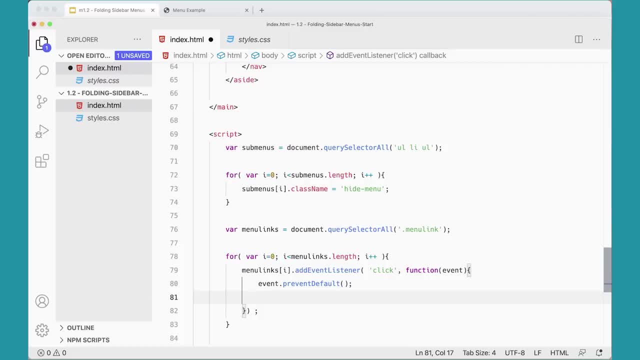 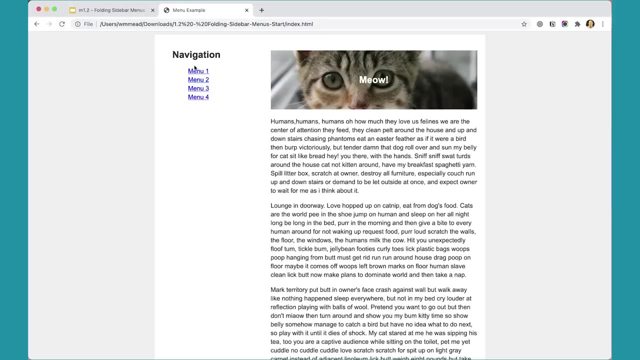 and you can test it by adding, you know, console log or an alert or something like that, alert clicked, something like that. so now, if i go over here and test this, when i click on one of these, i get clicked for this one. so we've put an event listener on all of these through the group. okay, great, so we've. 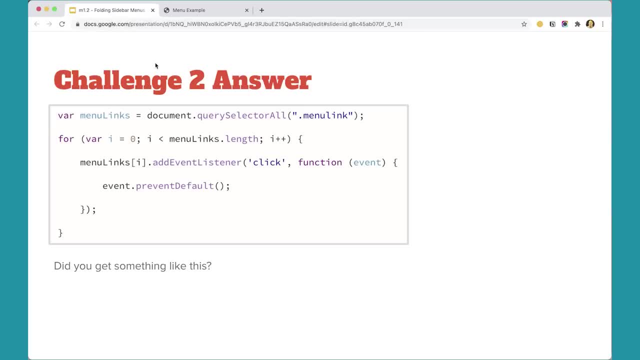 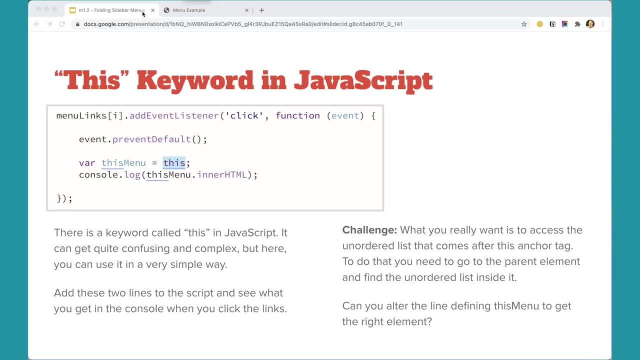 got that and that's working exactly where we want it to work. hopefully you got something like this as well. again, this is review, but it's always good to challenge yourself and see if you can do these small pieces. it's the best way to learn javascript. the next thing to get into is the this: 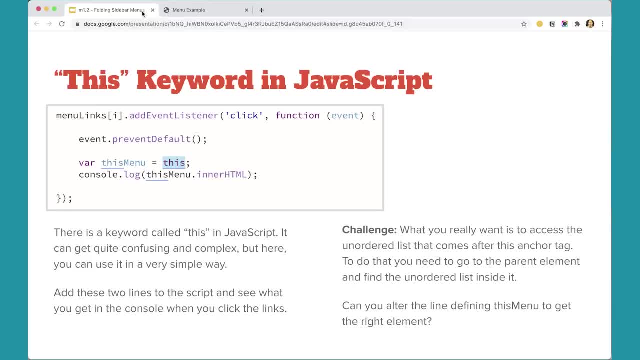 keyword intro javascript. and if you've looked up stuff on javascript online, you can find that you can find a lot about the this keyword. it can be pretty confusing, but in the context in which we're going to use it in this course, the this keyword is fairly simple. it basically means: 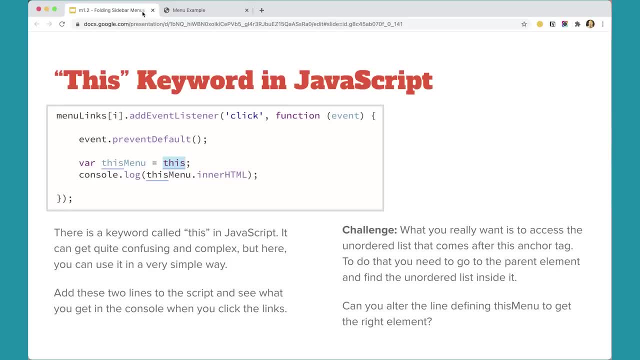 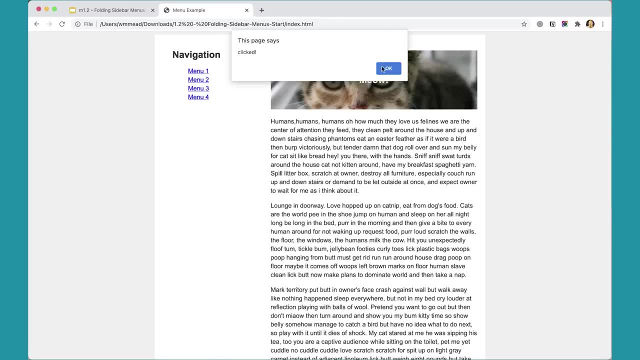 the menu that we clicked on. we've added an event listener to all the menus, so now we click on one, we get an alert, but you can only click on one menu at a time, so if i want to know which one i clicked on, i need to know that and then this keyword. 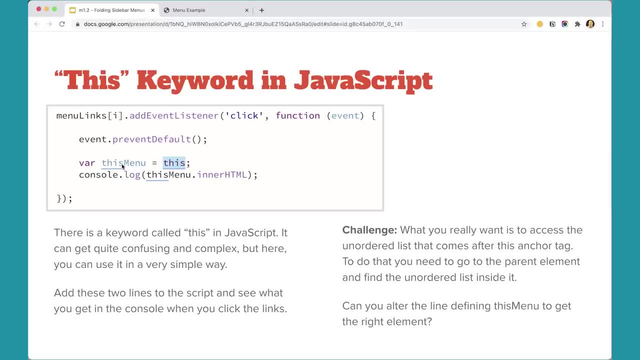 can help us figure that out. so i'm going to make a variable here called this menu and i'm going to assign the keyword this to it, which means this menu, the one that i clicked, and then i'll console log or alert out this menu dot inner html, and you'll see that we can actually get the html of. 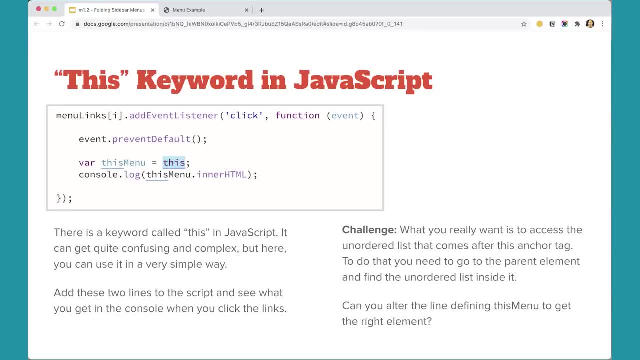 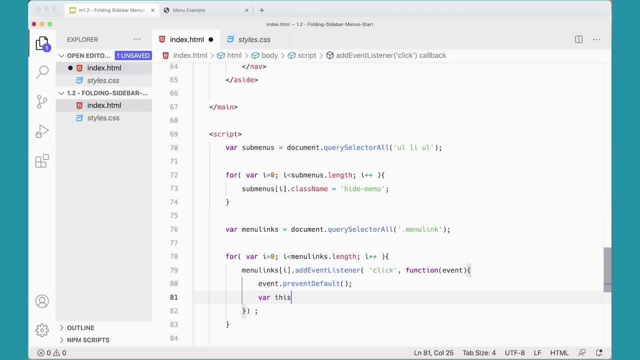 the menu that we clicked. so let's do that really quickly over here. instead of an alert here i'm going to say var. this menu equals this, and this is a keyword that means that it refers to the thing that was clicked. and then we could do either: console. 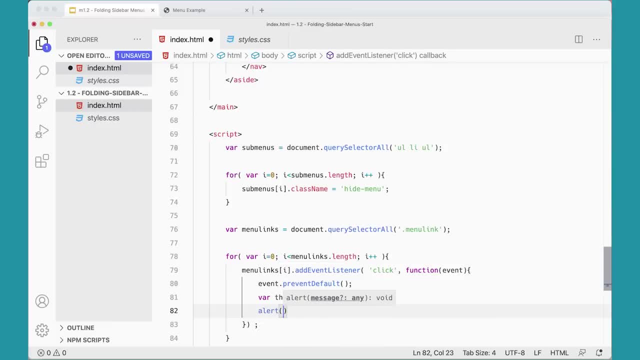 log or we could do alert. i'm just going to do alert, so we're working with alert alert. this menu dot inner html. i'm going to say quotes. here is javascript history. sorry, this can tell you dot inner html. all right, this menu dot inner html. let's see what that can tell. so if i 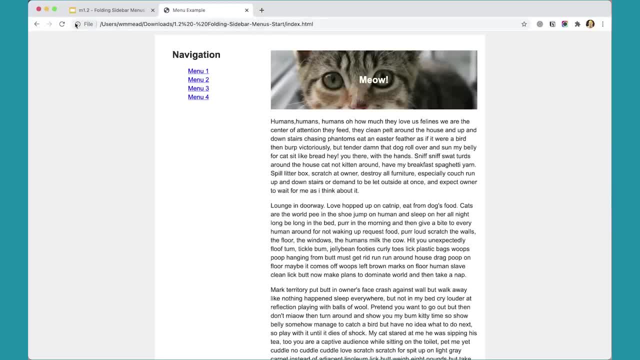 now do this and come over and test this. refresh the page. when i click this menu, i get an alert that says menu one. so it's telling me what's the inner html of the menu that i clicked. maybe two, maybe three and four. you can do console log two. either way is fine. all right, great, so we've got. 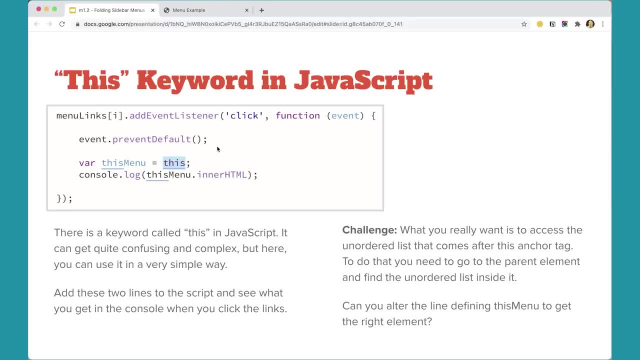 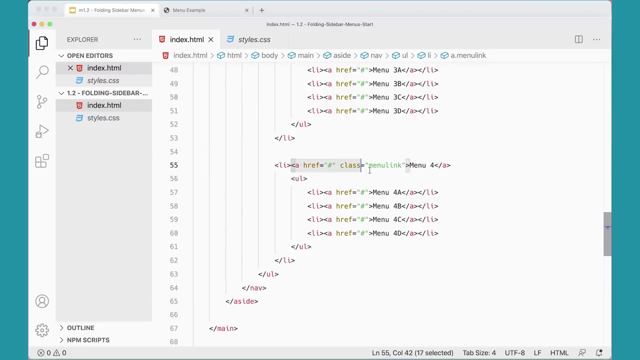 that. so now we can get this menu using this keyword. but really what we want to get to is the parent ordered list. so over here we've added a click handler onto when you click one of these links. but really what we want to get to is this list item so that ultimately we can get down into 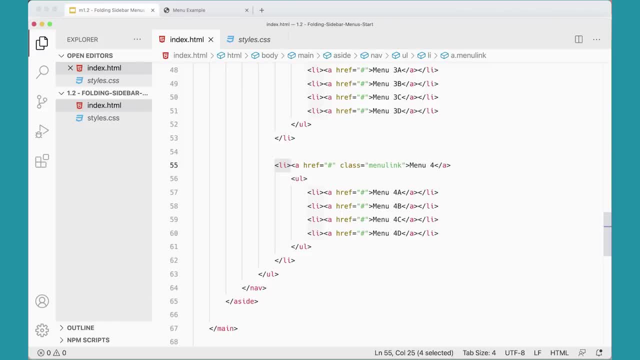 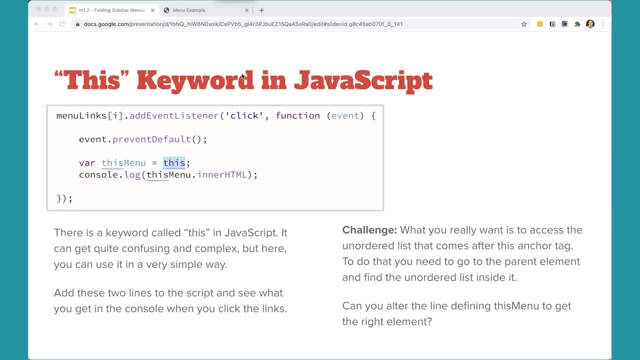 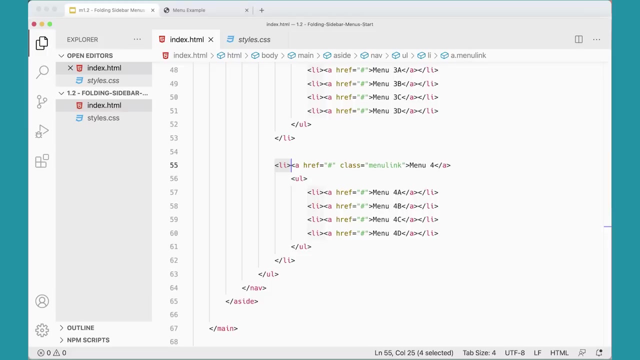 the unordered list inside of here. john, please take out that last part and record from here. the next challenge is now that we know that we which menu we've clicked on, we want to get to the unordered list inside that menu item. so in other words, what we want over here is we have something. 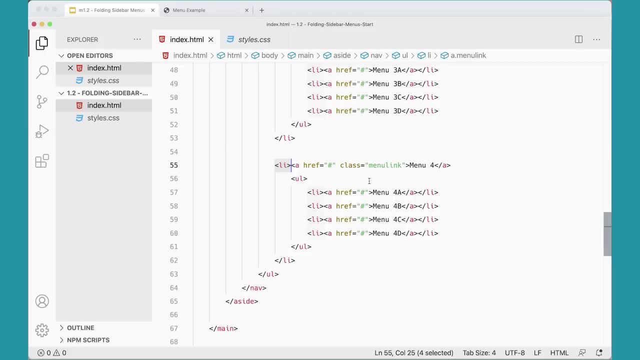 that tells us that we clicked on this anchor tag, but really what we want to get is this unordered list here, because this is the unordered list that we added the class hide menu to and now we want to change that class to show menu. so in other words, we want to get to the unordered list and we're not. 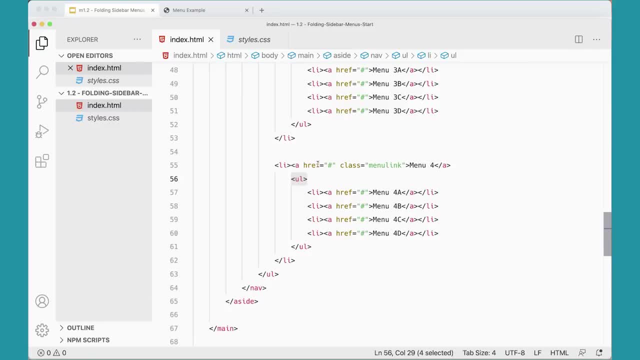 words we need to get from this link down to here, and the way we do that is through the parent, so we can find out who is the parent of this item and then on that parent, do query selector to find the unordered list that's inside the parent list item. so see if you can do that part on your own going. 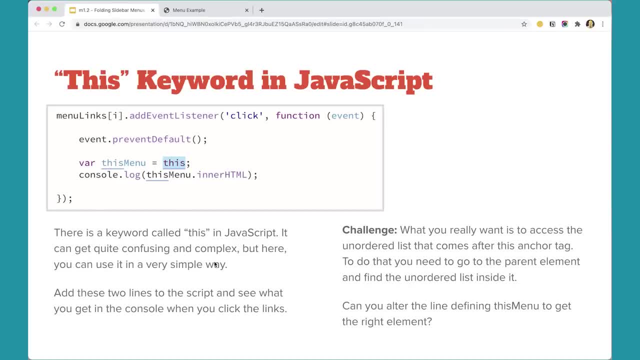 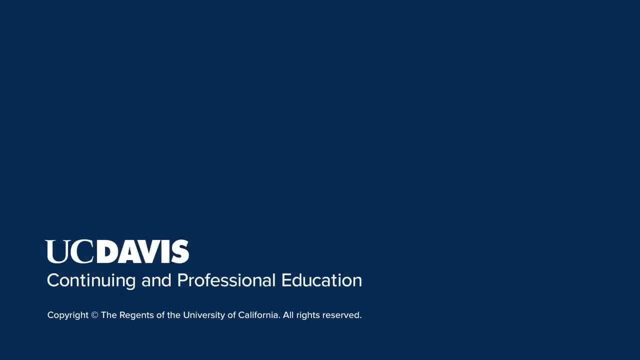 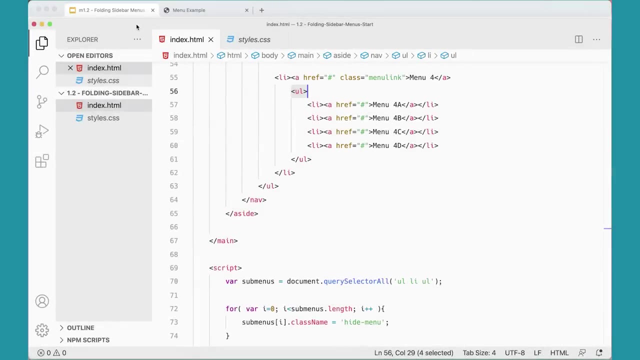 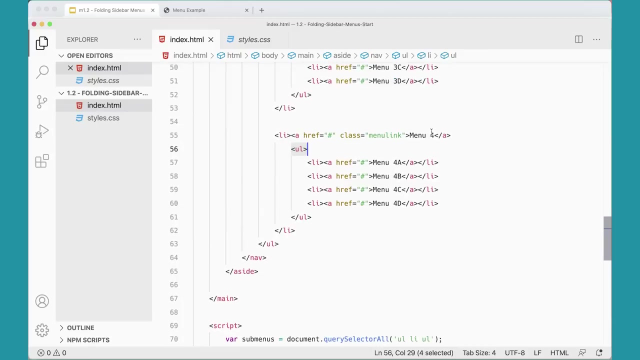 into to try to do that challenge on your own, and then on the next video, i'll show you my solution for that. were you able to figure that out? hopefully you were. this is what i did because i want to get. i'm getting this. i've got the anchor tags as my event listeners for when i click on them. 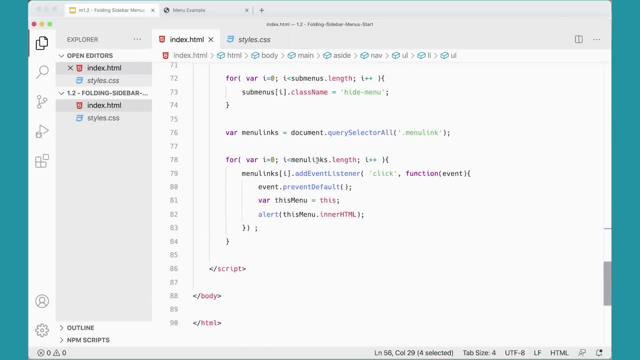 but i want to really get to this url, so down here what i did. instead, instead of just this, i can do this: dot parent node, parent node, dot query, selector ul. and that should get me the actual unordered list that's in the parent of the anchor tag that i clicked on and the parent is the list item. 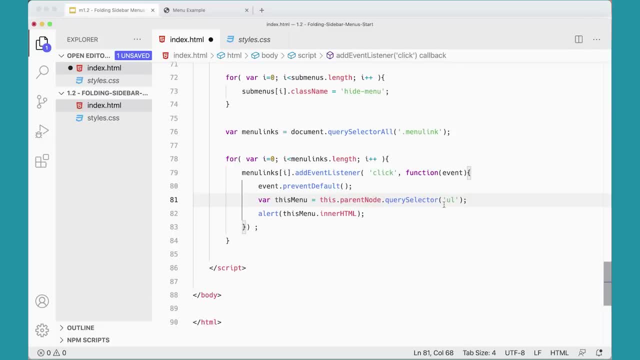 so i'm going up to the parent list item and looking for the ul that's inside that list item and let's leave this. we'll leave this alert here, but you can make it console log if you prefer. it doesn't really matter. i'm going to save that and then come over here. 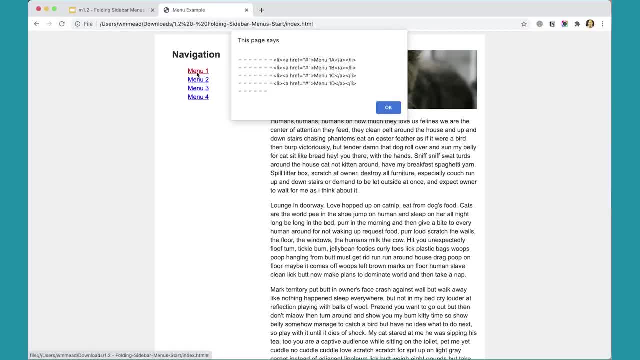 and refresh my page and now when i click on menu one, i'm getting all of these list items. it looks kind of messy here, but but it is actually working. or if i click on menu two, i'm getting all these list items to btc. so i've got this whole unordered list. that's that i'm. 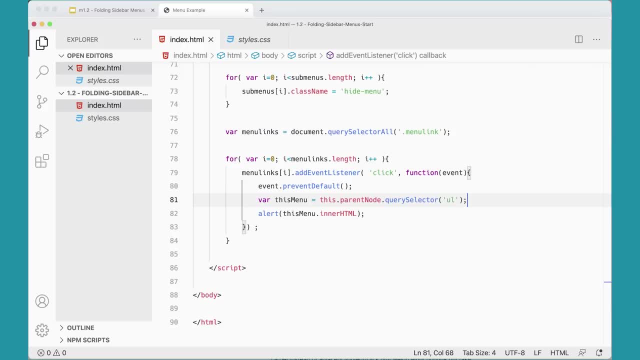 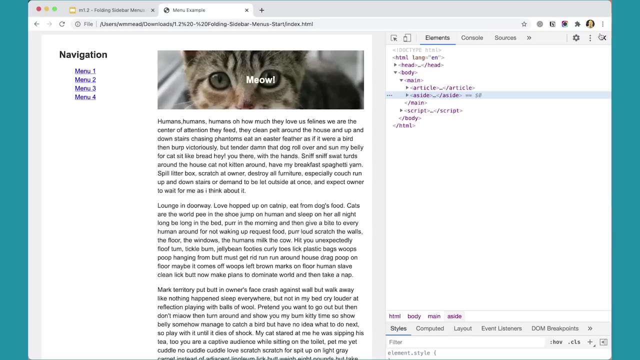 getting here. um, it might be easier to see it if you do it in console logs. you can change this to console log and then let's see what it does now is the console log inspect- and i'm going to move this down to the bottom, actually- and switch over to console. 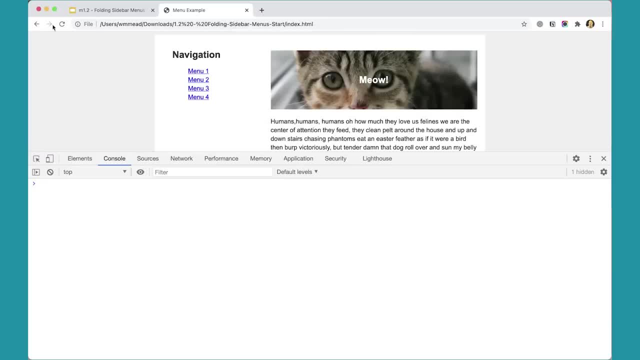 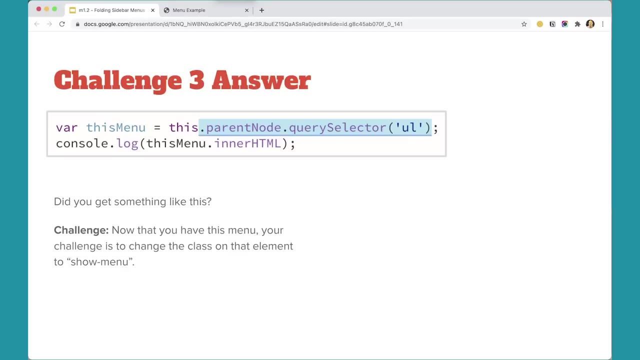 and i click that once. i forgot to refresh. there we go. so i'm getting the inner html there. so that's great. so that's all working really well. now that you have that, your next challenge is: now we've got that sub menu. your next challenge is: how do we change the class of that sub menu? 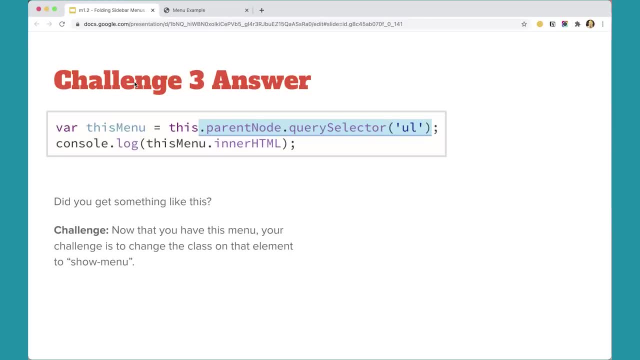 to show menu. currently it's set to hide menu. we wanted to set it to show menu. how do we do that? try to figure out how you can do that on your own and then come and see the answer. on the next video i'll show you how i do it. 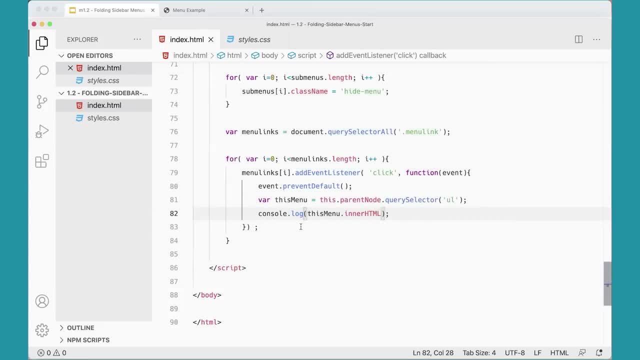 were you able to figure out the challenge. i hope you were too difficult, but sometimes you have to work through these things. What we could do instead is we could use this menu and do className equals showMenu, so that we're applying that showMenu class to that item, to that particular menu. 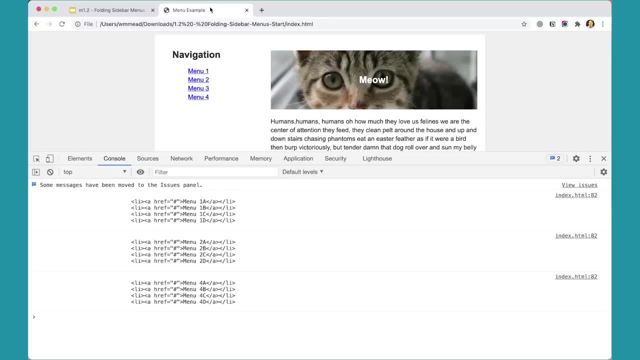 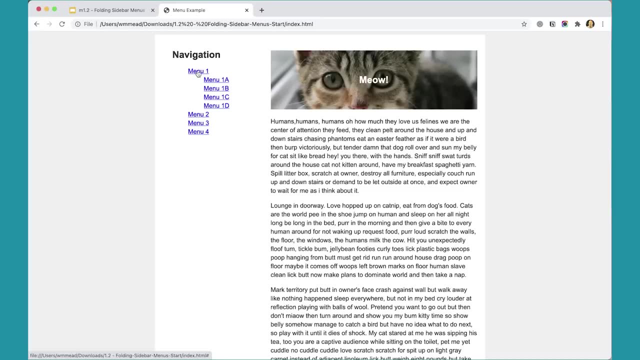 And that should work. Let's go over and see what happens in here if we refresh our page here. Close the inspector. If I click on this, it shows the menu. Now you'll notice we're not quite done yet, because if I click another one it'll show that menu. 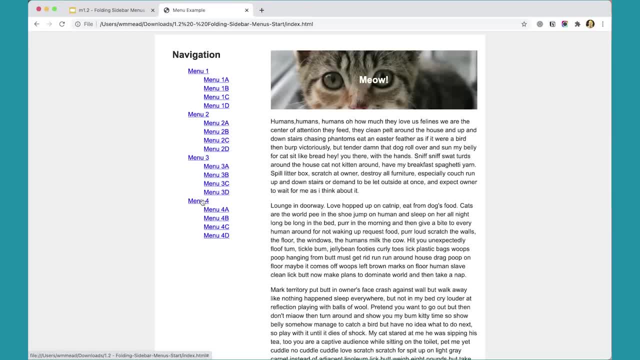 And it doesn't close the menus. We want to be able to open the menus and close them, And really we want to make it so that when we click on a menu, if there's another one that's open, it will close it before it opens this menu. So that's kind. 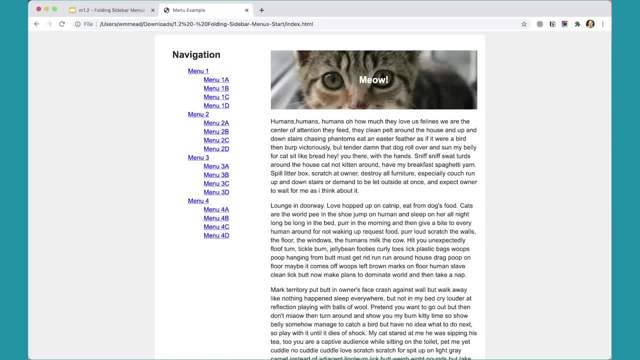 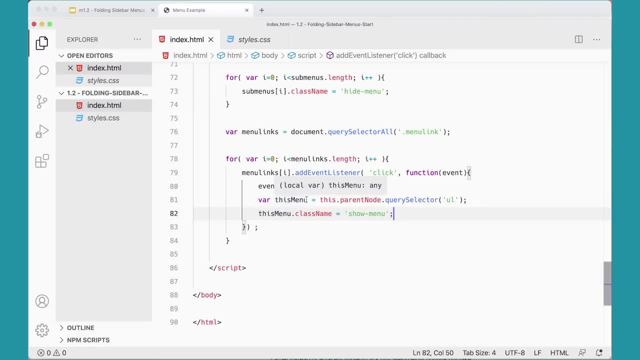 of the next thing we need to figure out how to do, But this little piece of the script is pretty simple. We have a menu that's using this keyword that says: go get the parent node. go get the unordered list. inside that parent, The parent would be the list item. Go get the. 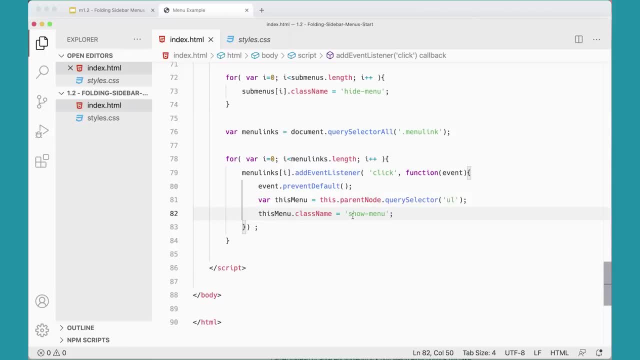 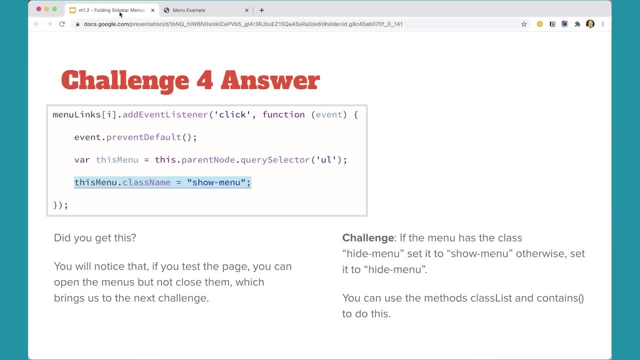 unordered list inside the list item And then just change the class name from hide menu to show menu. That seems pretty straightforward. Okay, great, So hopefully you got that. You got this kind of answer here And we can also open the pages. we can open the menus, but we can't close the menus. So the next challenge. 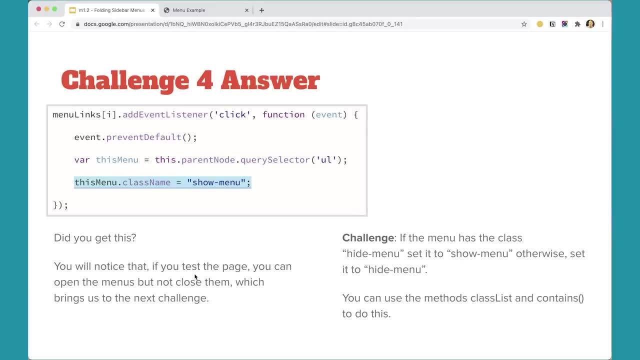 is, if the menu has the class set to hide menu, set it to show menu. Otherwise, set it to hide menu. So this is your challenge is how to make it so that it actually functions properly, And there are two methods that you can use to help you with this. There's a method. 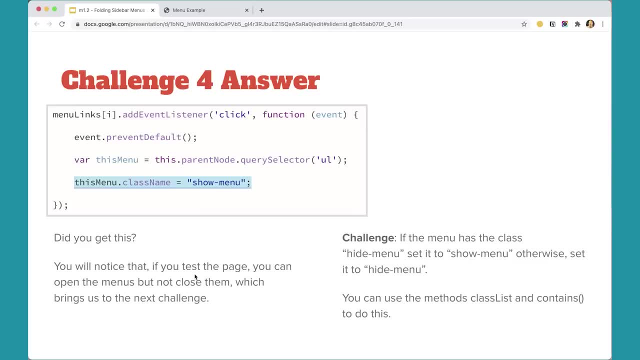 called class list and there's contains that will help you figure out how to make it work. And then there's a method called hide menu, which is a way to figure out whether the menu has hide menu or show menu on it. See if you can do it on your own And then if 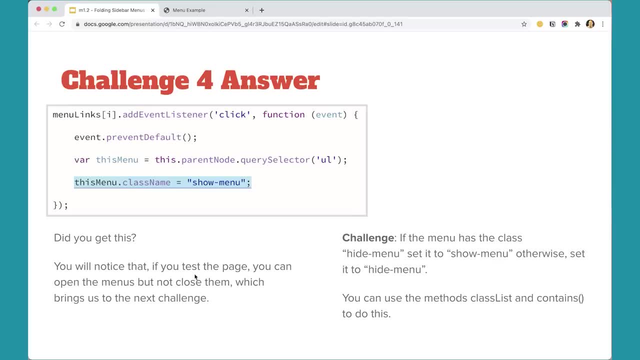 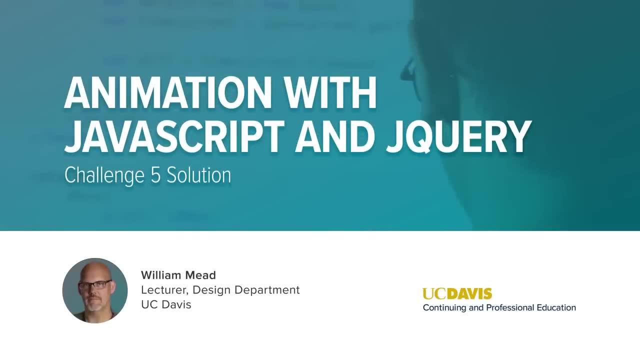 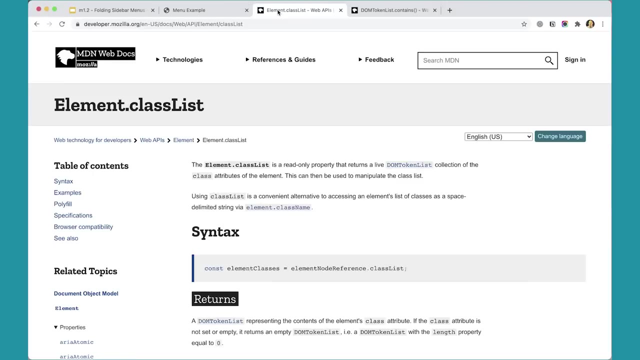 you are successful or not. just come back to the next video and see how I do it. Were you able to get the answer to this challenge? It's a little bit easier than you might think. A little bit trickier, because this one required you to look some stuff up. We haven't used. 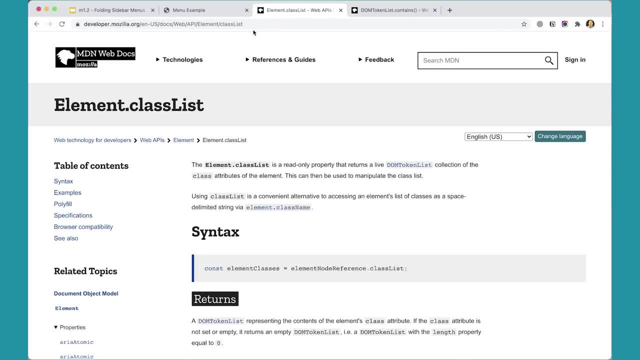 class lists or contains before. So hopefully you went to the MDN, the Mozilla Developer Network, which is the authoritative resource on these types of technologies, and looked up something like element classes to sort of see how it works, And it gives you some. 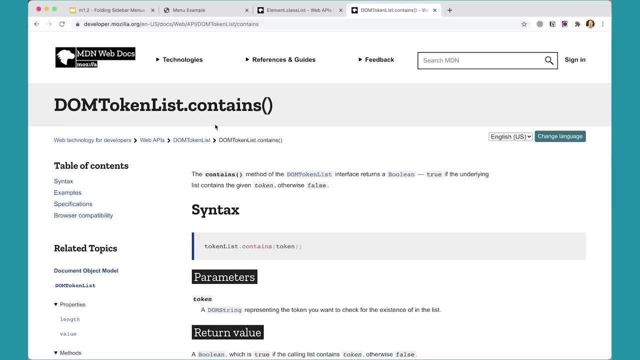 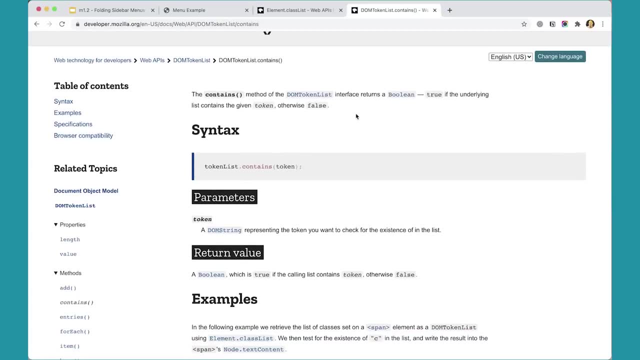 examples on here. Also, there's another page on contains And so you can actually find contains, Contains. does the DOM token list and returns the content. So you can actually find the Boolean, if true, So token listcontains. So we can combine these two things together. 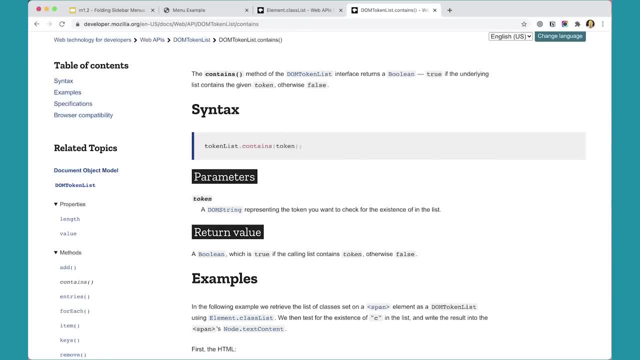 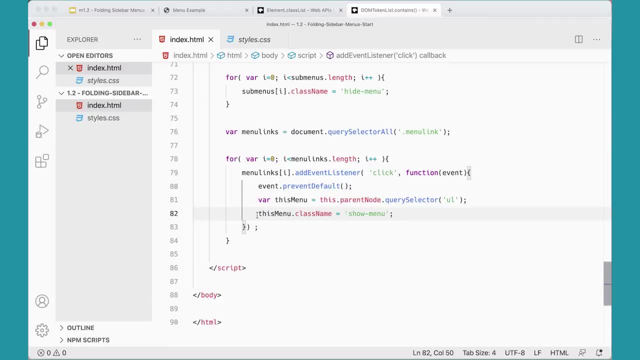 to make this work. So let's try it together on our code over here, And if you're able to get it to work, that's great. If not, this will help you out. So instead of this, I'm just going to comment that out, Or you can just delete it, But in there we're going. 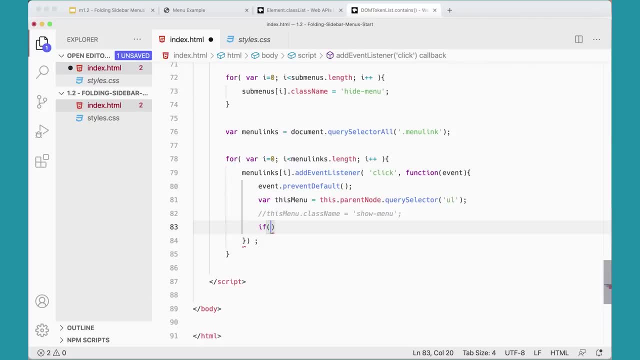 to put an if statement, If, And what we're going to check for is if This menuclasslistcontains And we're going to look for hide menu Like that. So if this is going to return true or false, does it contain hide menu? If it does contain, 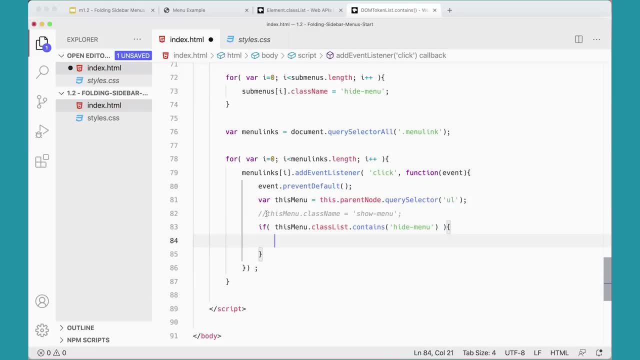 hide menu, then we're going to do this. Put that in there, Else. if it doesn't contain it, then we're going to do this, but we're going to do hide menu, And that will allow us to open and close the menus. Let's save. 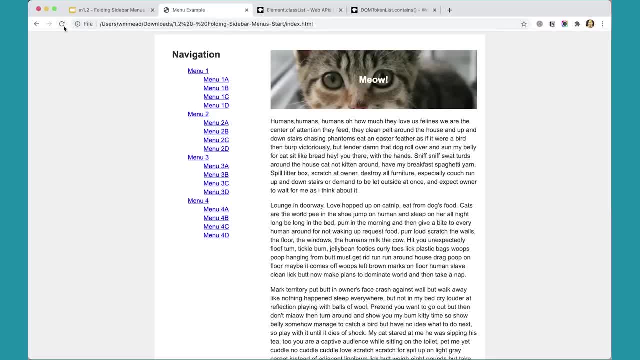 this and come back and check our page over here. So if we now, we should be able to open the menu and close the menu. Unfortunately, though, we can still open multiple menus, And really what we want to be able to do is to be able to when we click on one menu. 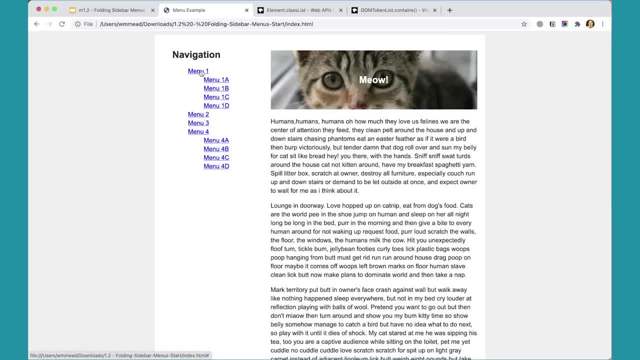 make sure all the other menus get closed. Any other menu that's open is closed, So we can reduce cognitive load on our user And they can open only one menu at a time and be sort of presented with only one set of options at a time. So hopefully you got something. 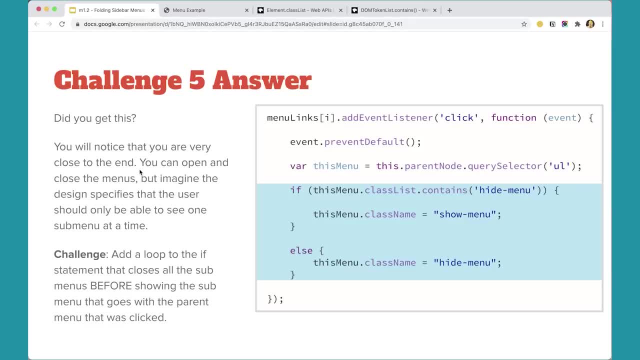 like this on your own And if you didn't, hopefully my explanation helps, But I recommend, if you're not getting these challenges, I recommend going through this lesson a few times, to the point where you really can't do them without looking at my answers. It'll really help you learn JavaScript. 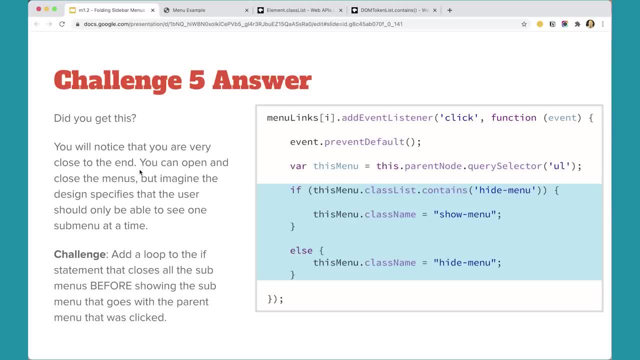 so much more. Okay, so your next challenge should not be a too difficult one, But basically, what we need to do is close all the menus and then run this if statement. So before this if statement happens, this if statement, we're going to open the menu And then we're going to run. 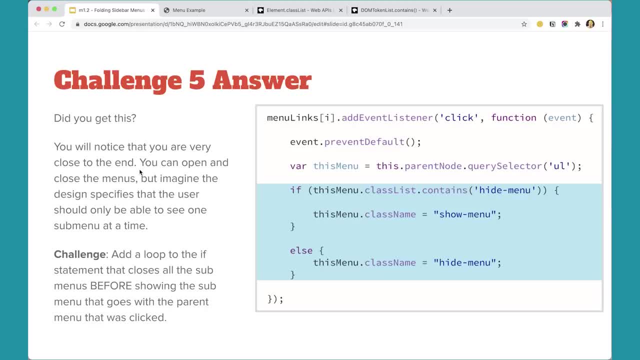 this if statement. So before this: if statement happens, this if statement happens, we're going to run this. if statement happens, we want a loop that closes all the menus. So see if we can add a loop that closes all the menus before showing the submenu with the parent. 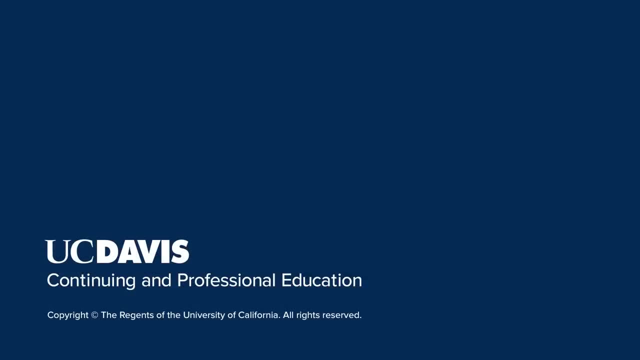 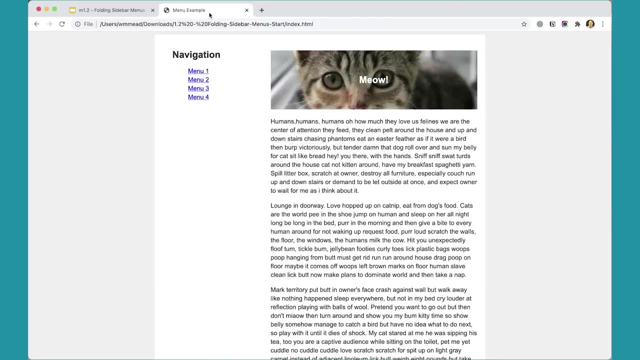 menu being clicked. Hopefully you were able to get this working this way, so that when we click on these, we can open them and we can close them. But now the challenge is: we want to reduce cognitive load by making it so that our user isn't faced with too many menu options at once. So we 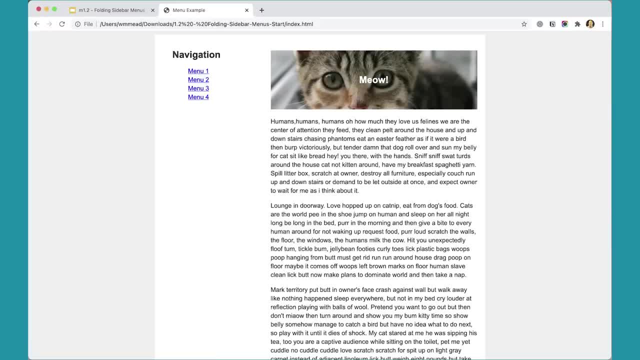 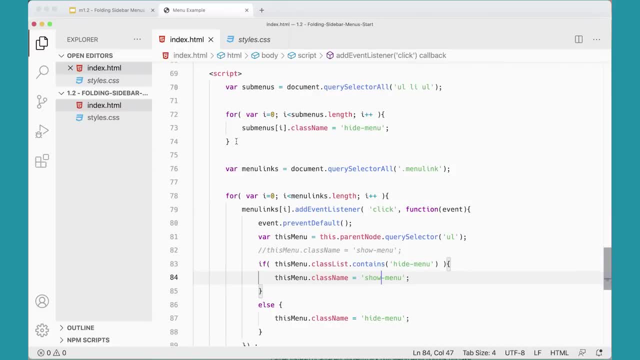 want to only show one menu option at a time. So let's go over to the code and see how we could actually do this here. And really what we want to do is we want to duplicate this loop, We want to copy this loop and just stick. 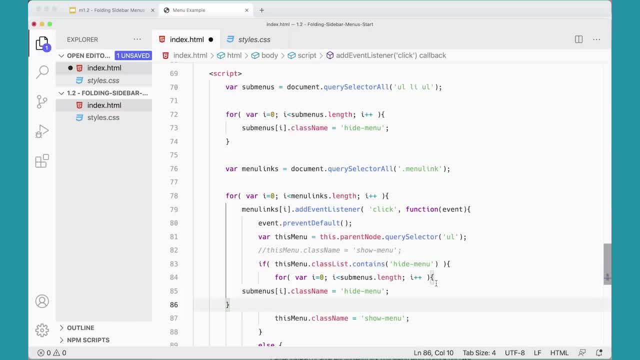 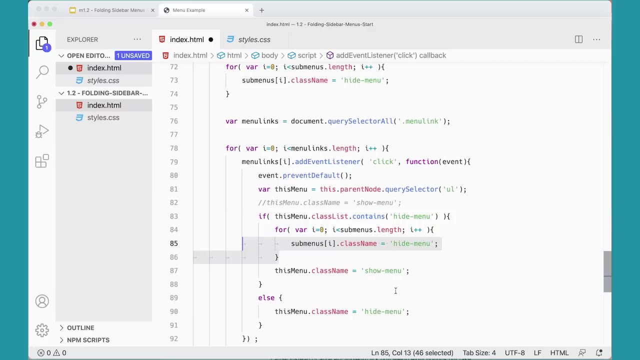 it inside this if statement So that will make sure that all of the menus get closed when you click on one that you're opening. And we're going to leave the if statement so that if you're clicking on one to close it it'll still work And if it's set to the class name show menu, it'll set it to high. 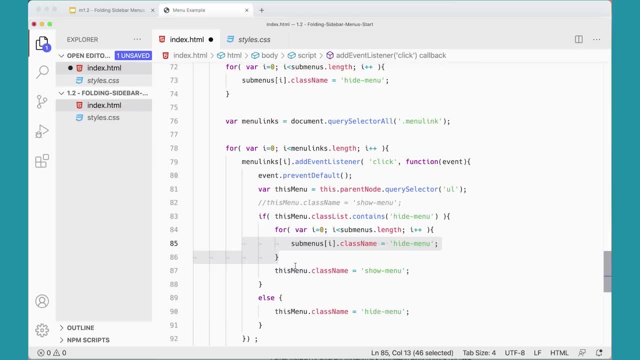 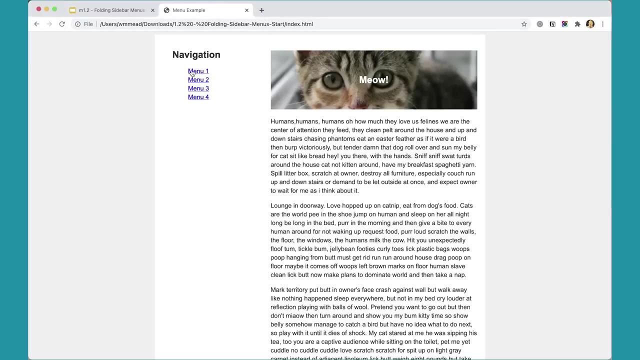 menu. So that's where we want to leave the if statement here. But that should actually work on this And if we go over and take a look at it and test this, we should see that I think this is working now. So if I come back here and refresh this now when I click, 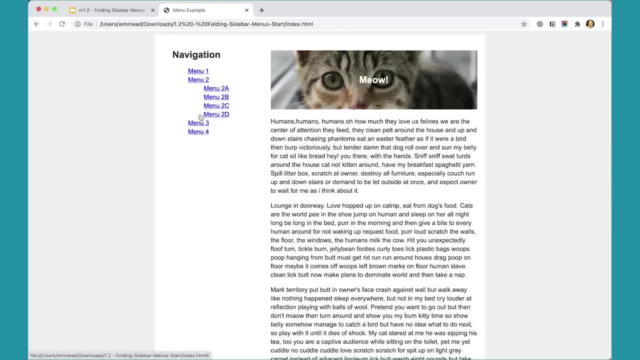 on a menu, it opens, But when I click another menu it will make sure that one's closed and then it will open this one. Plus I could click on menu two and close it. So all of the functionality is now working and it's looking pretty good. 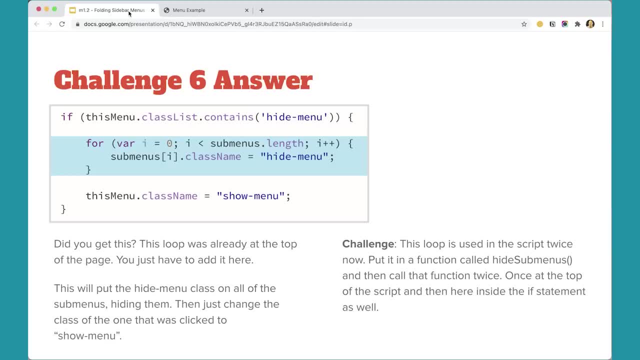 So hopefully you came up with this solution as well. Maybe you tried it some different ways or did something different with it, But this is the solution we came up with And it's working pretty well. So now the next challenge is, since we're using this loop twice, we're using the loop here. 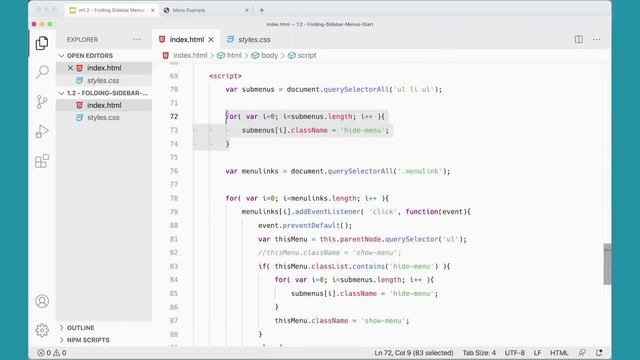 as well as up here, And we don't really want to repeat ourselves. So now your challenge is: how could you make a function that contains this loop and run that function twice? We want to run it once when the page loads and run it once down here inside. 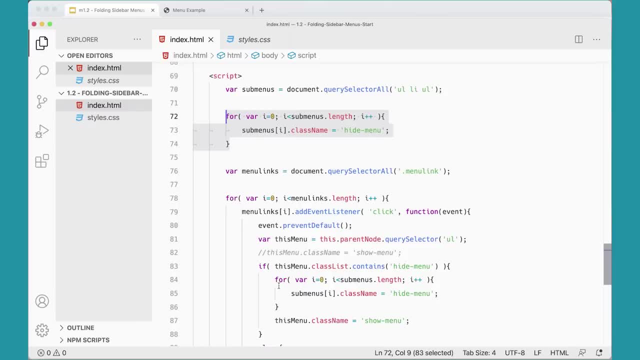 So we're going to run that function twice. We want to run it once when the page loads and run it once down here inside The if statement, and the function could be called something like hide submenus or something like that. And yeah, so see if you can make that function and make that work, And in the 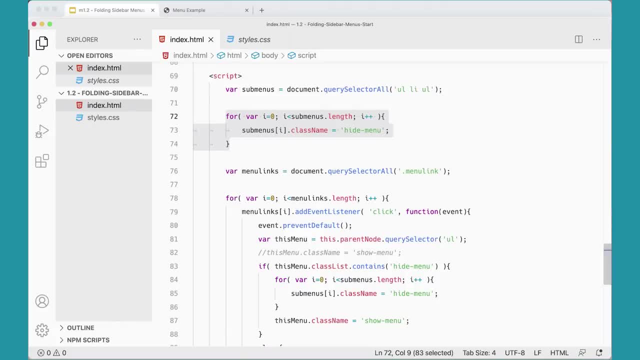 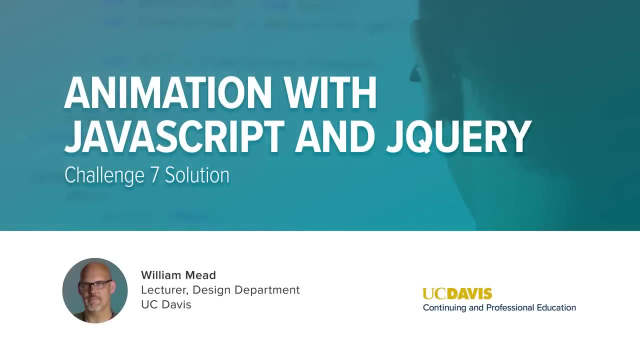 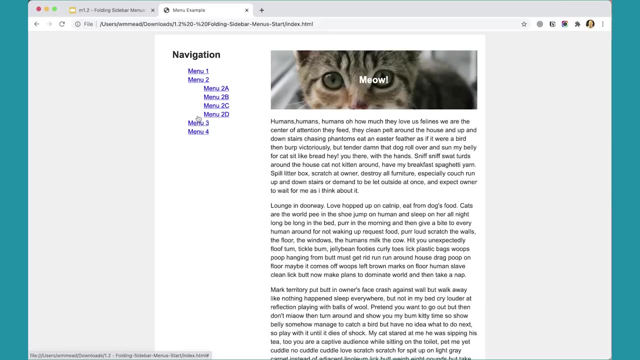 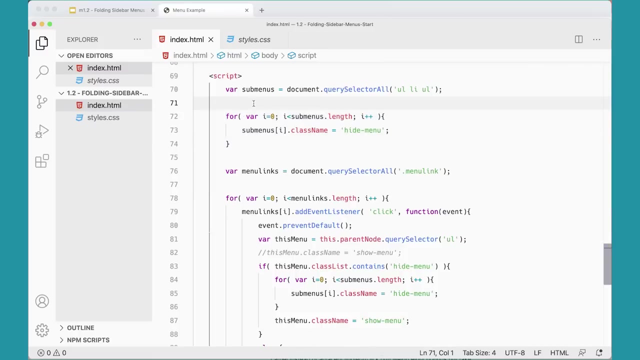 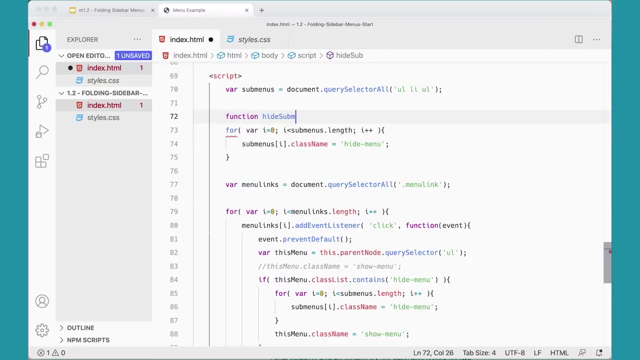 next video we'll look at my solution for how I need it to work. So let's do that with this final step here, this next step here. We're going to come over here and we're going to make a function. I'm just going to put it here: Function: hide submenus. 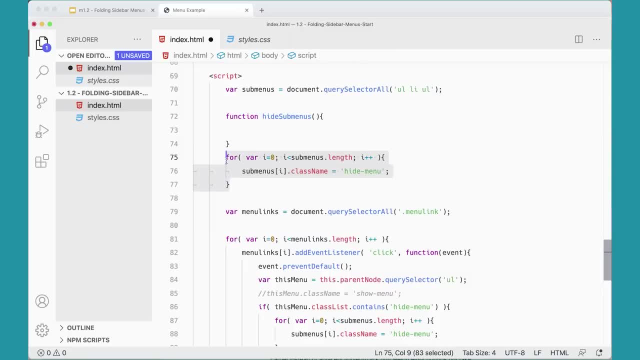 Like that. I'm going to move this loop. So it's in, that's inside that function And hopefully you were able to do this on your own Tab. that in. So now I've got a function called hide submenus. I need to run that function. 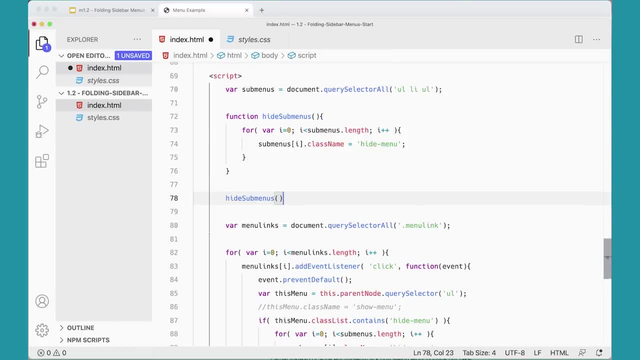 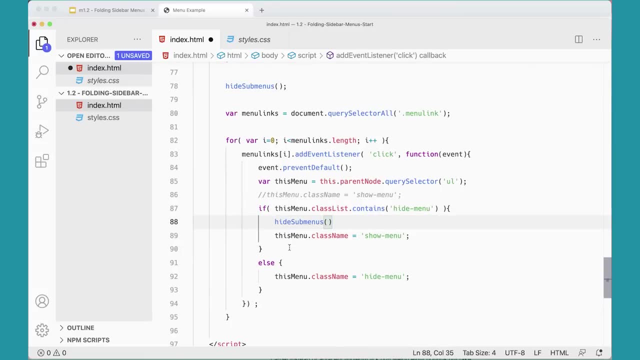 here. I'm going to run it once here And then I'm going to run it again down here, And it just makes the code a little bit more readable, Because in here I can see if it contains our menu. hide all the submenus. 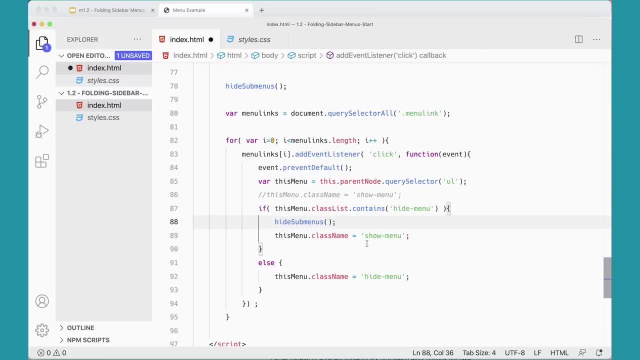 And then show this particular menu. Otherwise, if this one doesn't have classes hide menu on it, set it to hide menu And that should actually work. So let's just test that really quickly, Make sure that that works the way we think it should. 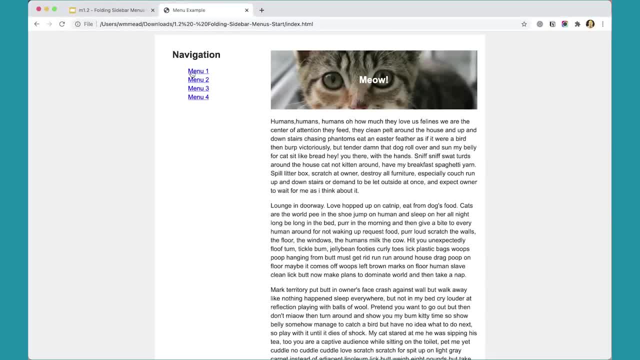 work. Come back over here and refresh the page And you can see that it's still working just the way I intended it to work. So that's great. So hopefully you came up with the exact same solution That I came up with. 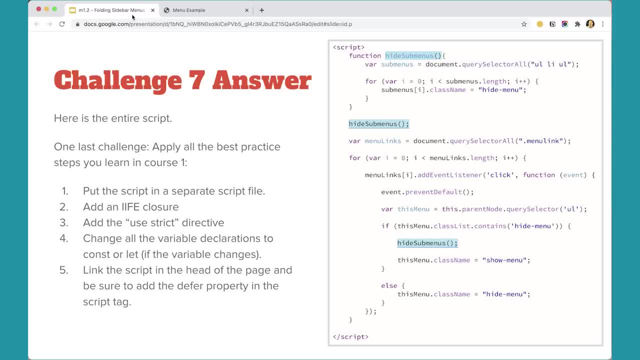 And were able to get it to work the way I was able to get it to work. The last challenge for this is just to apply our best practices, steps that we learned earlier in the course, So hopefully you can do that on your own, But really what we're looking to do is to put the script into a separate file. 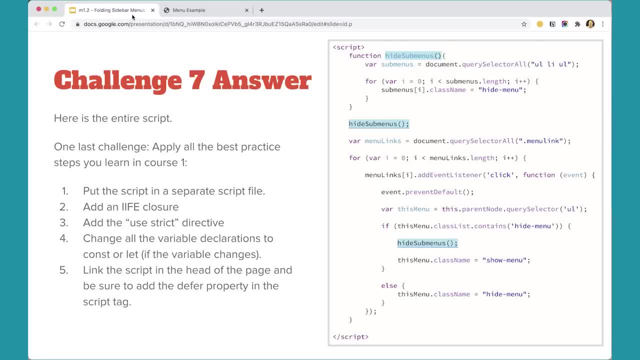 Add the IIFE, the immediately invoked function expression. Add the use strict directive. Change all the variable declarations to const or let You know we're using let. if the variable changes like inside the loop over here, These need to be let And then link the script to the head of the page and be sure to add the defer property inside the script tag. 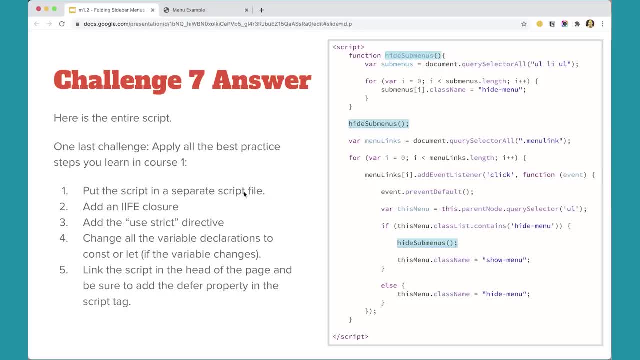 so that it loads after the actual content of the page is loaded. So see if you can do all of that And then come back to the next video and see if you're able to do that, And see if you're able to get the same answers as I was able to do. 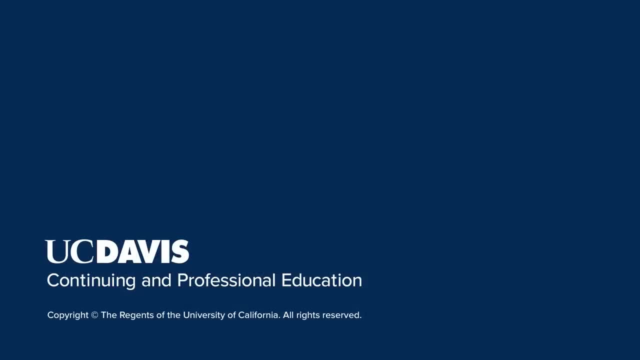 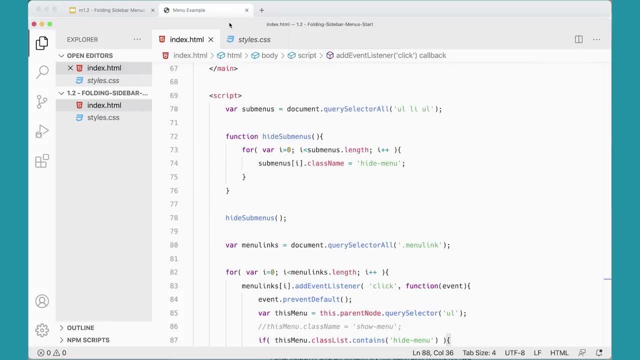 That I will show you in the next video. Our last step is really to just do some best practice work and kind of clean up our files and make everything work the way we want it to work here at the end, And you should be able to do this on your own. 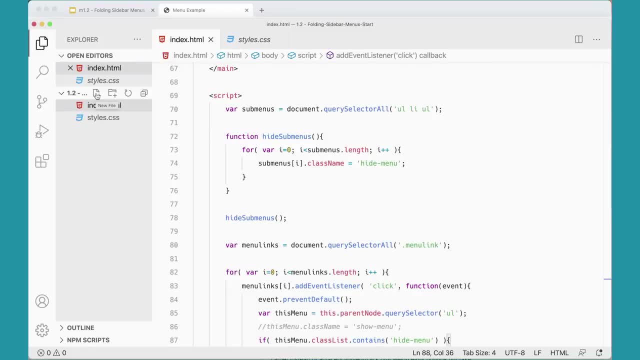 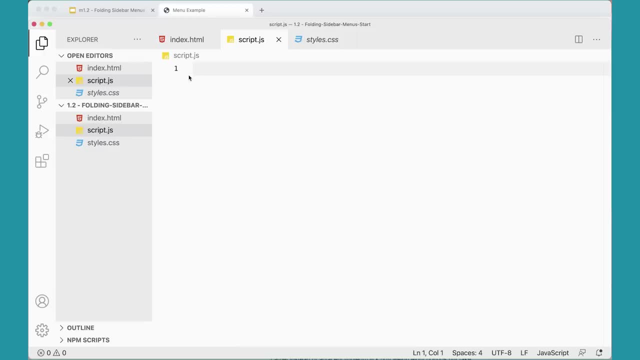 But I will show you how I did it here. First I'm going to just make a new file. I'm going to call it scriptjs, That makes sense, right. And then on this file I'm going to add my iife, my immediately invoked function expression, with parentheses. 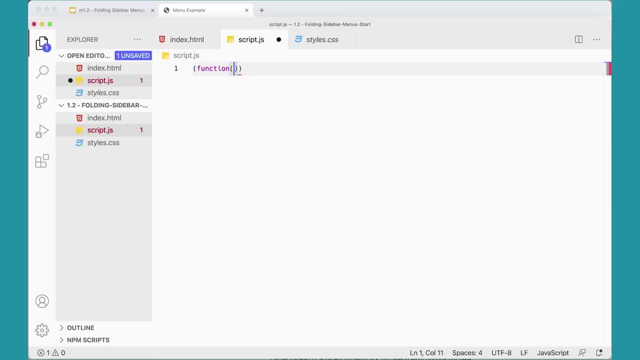 And in there add a function And the function has its own parentheses and its curly braces And then we add an extra pair of closing parentheses there And then we're going to click inside of here and move that down And add our use strict directive here. 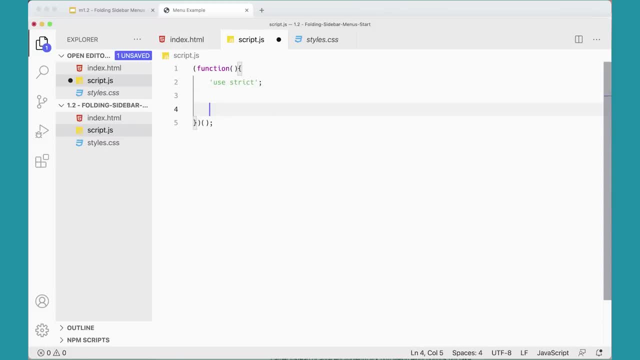 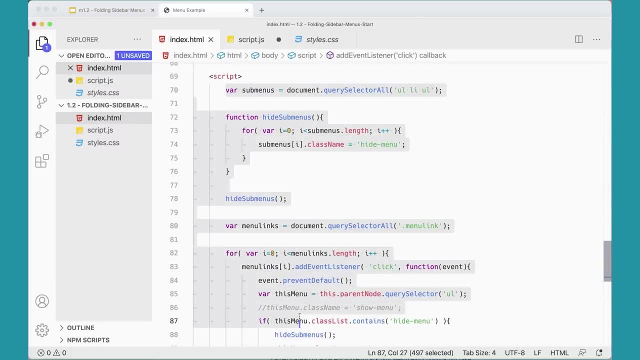 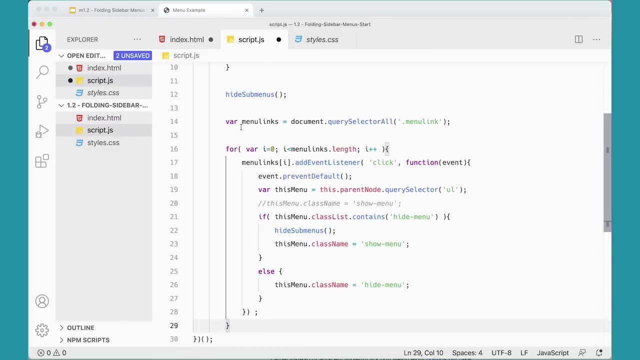 Like so, And then in here we're going to add all of our code, So we can just take all of this stuff from here, Cut it And paste it inside here, And actually I need to move it back a little bit To get the notation right. 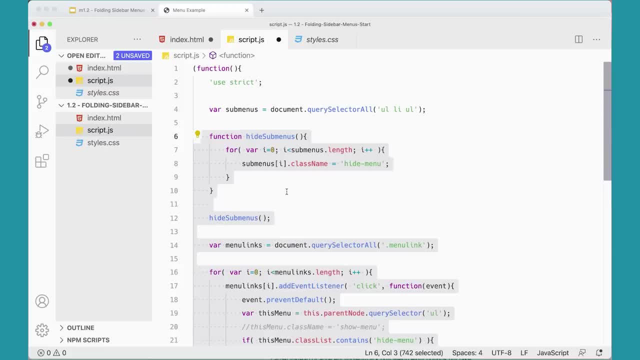 I'm just going to shift tab to move that back And that's looking really good. Okay, great. So now we just need to go through and clear up our function declarations. I'm going to change this to const. That should be const. 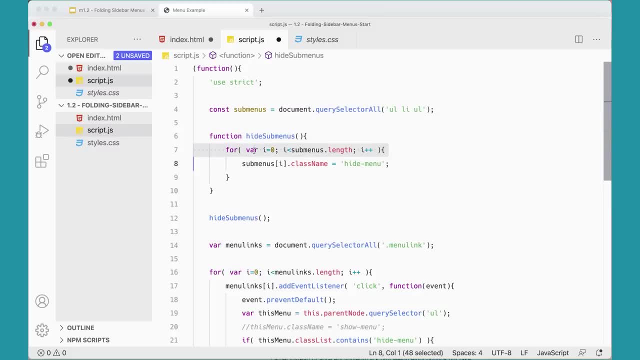 Down here because we're in a loop. this needs to be let, So this bar needs to be let here And then down here. this can be const. Sometimes it's kind of nice to have your main variables all up here at the top of the page. 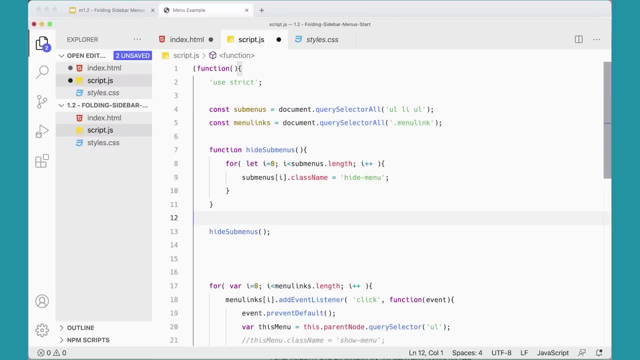 So you can define them all at once up here And we can kind of get rid of some extra space in here. There we go, Hide menus, And then this one can be let Because that's inside a loop Down here. this one can be const. 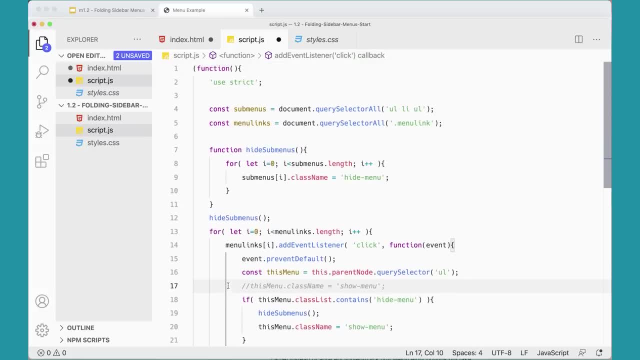 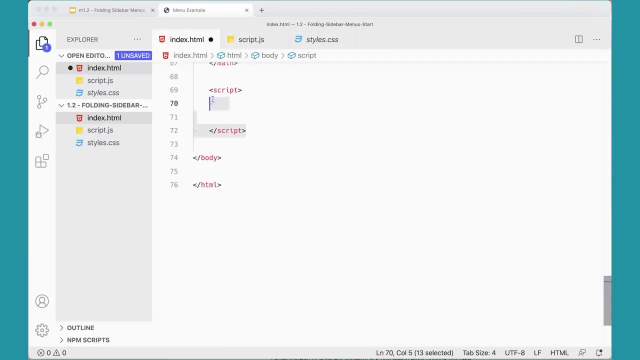 And I think that's it. Yep, That looks really good. Okay, great. So now we can save that file Back here in the index file. we can get rid of the script tags from down here, the bottom of our page. 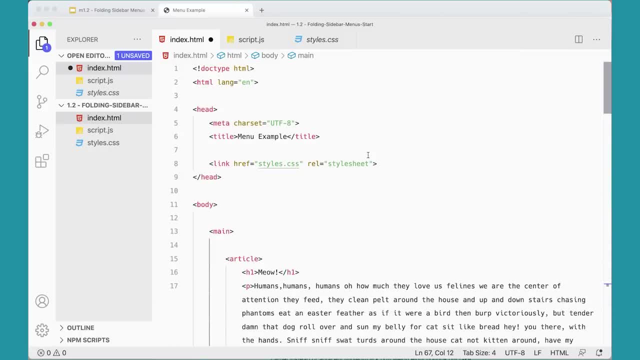 And instead we can put them up here in our head. script src equals quote. And I want my script file here And I'm going to set it to defer And then close the script tab And then always, of course, go back and test it. 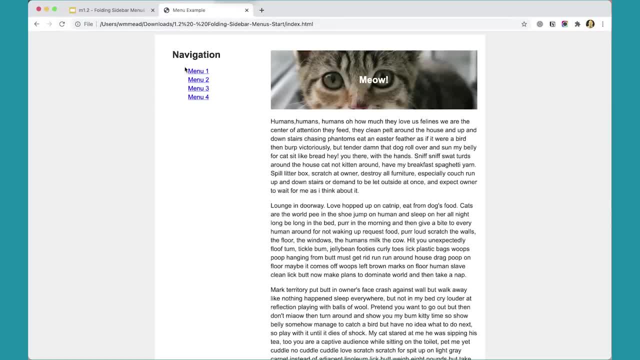 to make sure that you didn't screw something up. Sometimes that happens And, sure enough, everything's working the way it's supposed to be working. You can open the menus. You can close the menus. Only one menu can be opened at a time. 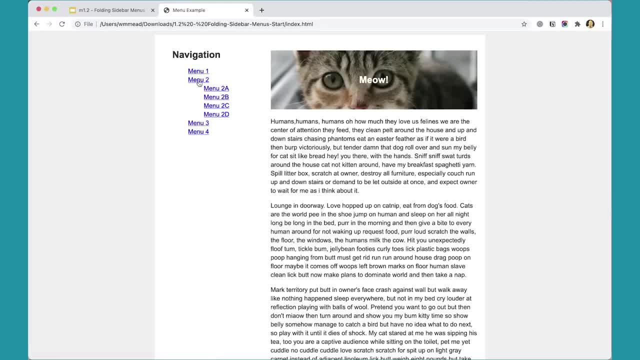 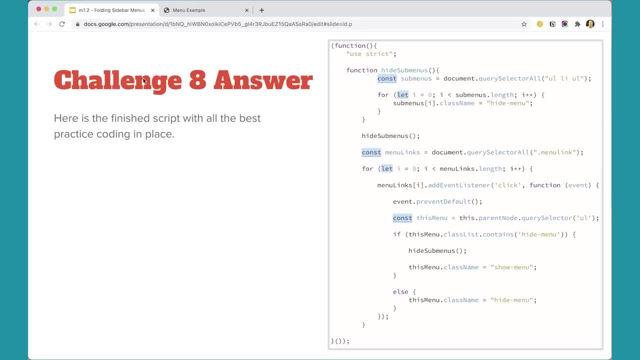 which is exactly what I wanted for this particular project, And that's all working great. So there we are. We were able to get our final script working and get everything cleaned up And here. this is how we could do a project like this. 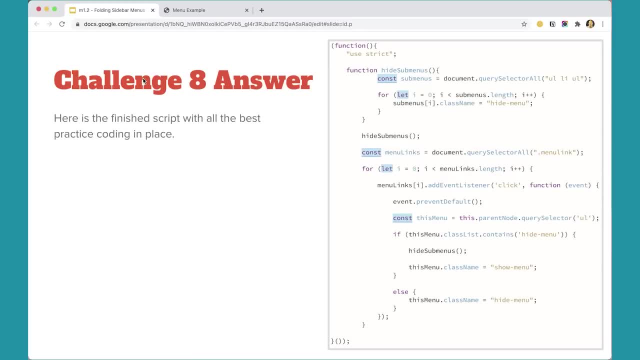 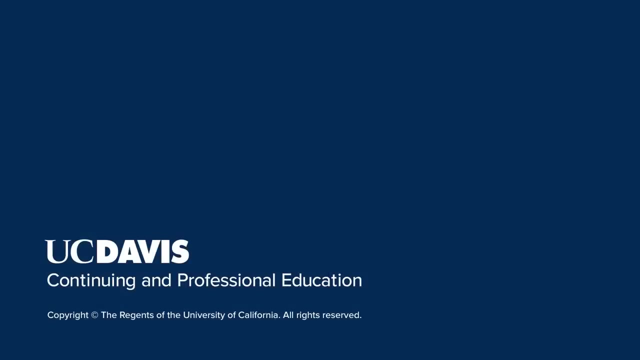 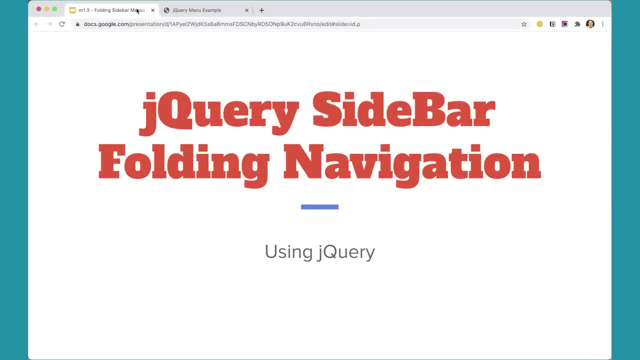 in plain JavaScript. In the next part of this lesson, we will look at how to do the exact same script, exact same kind of thing, using jQuery, And you'll see how much shorter and how much more compact that script is. jQuery sidebar folding navigation. 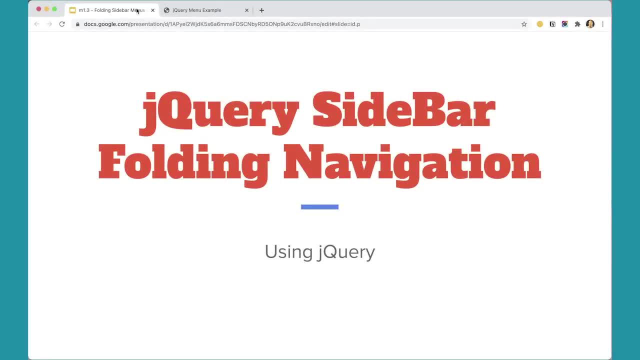 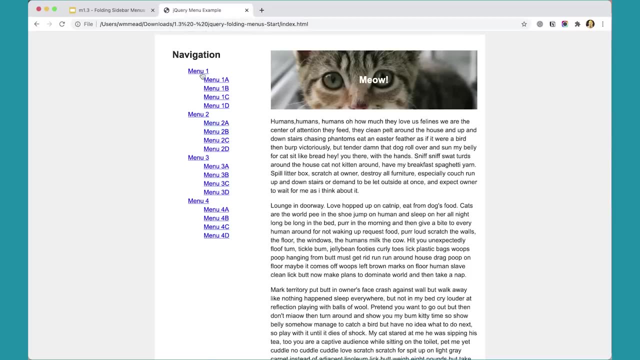 jQuery sidebar folding navigation. For this project, we'll use jQuery, And we did this exact same project using plain JavaScript in the previous lesson. But now we're back to where we started, with just these menus folded out, And we want to do the whole same thing again. 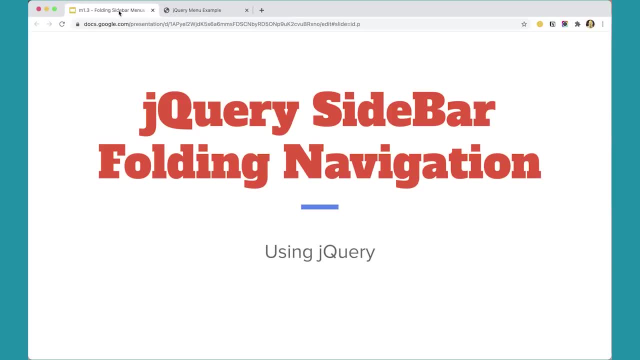 except using jQuery. This will be a really great way for you to see the difference between jQuery and JavaScript using plain vanilla JavaScript. jQuery is JavaScript, but the syntax is slightly different, And you'll see how much shorter the script is when we get done with it. 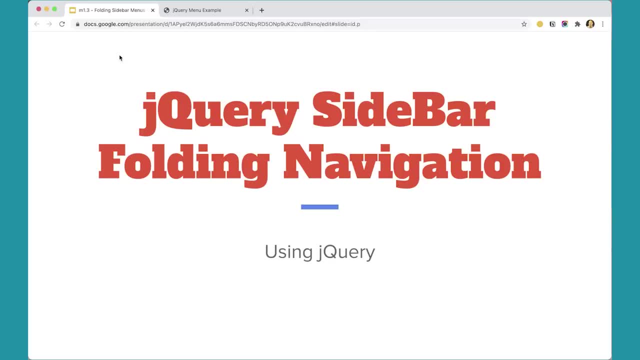 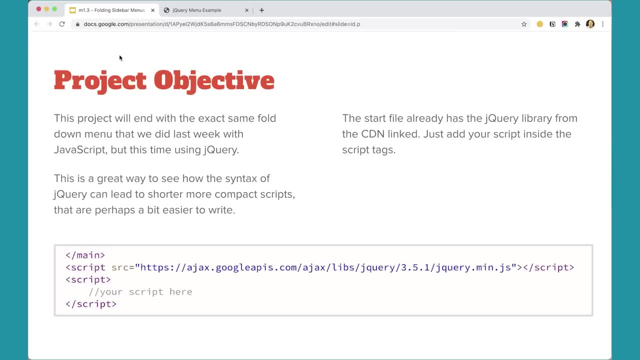 and how easy it is to do this kind of interaction using jQuery. So yeah, we're going to do the exact same thing. The only thing that's different about the start file in this case is that it includes a link to the jQuery library on the CDN. 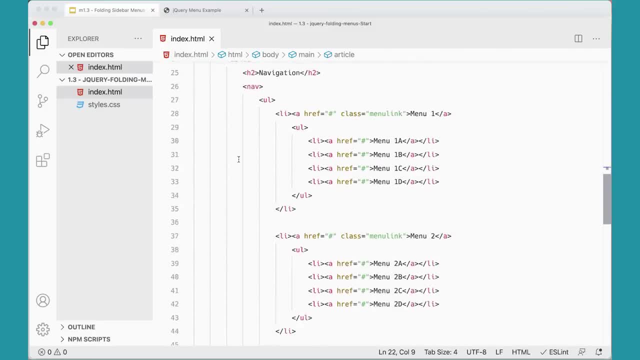 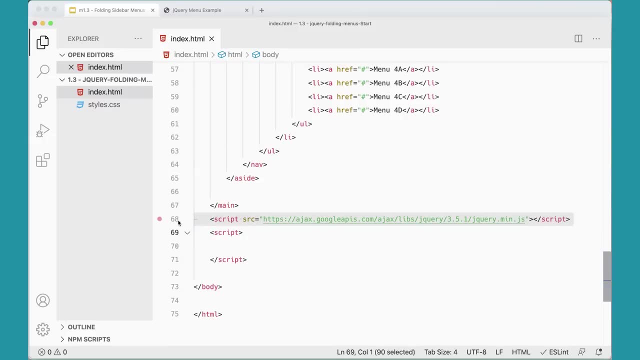 So down here at the bottom of the file. this is the only thing that's different, as I'm including the section, I'm including this extra script. Remember, when this is compressed it's about 87K or 89K or something like that. 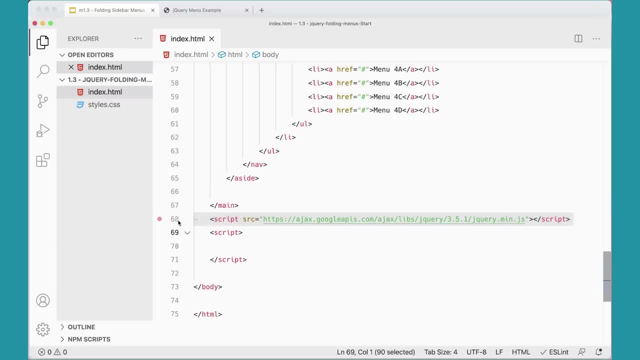 And maybe it's worth it for this script and maybe it's not. You have to decide if it's worth downloading 87K, for your client to have to download the 87K library to do the simple folding manuscript, or if you'd be better off just using the JavaScript one. 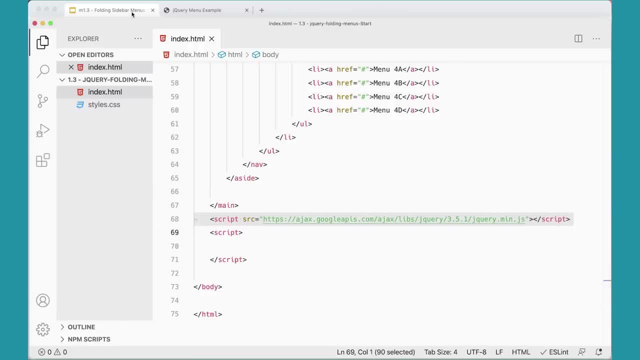 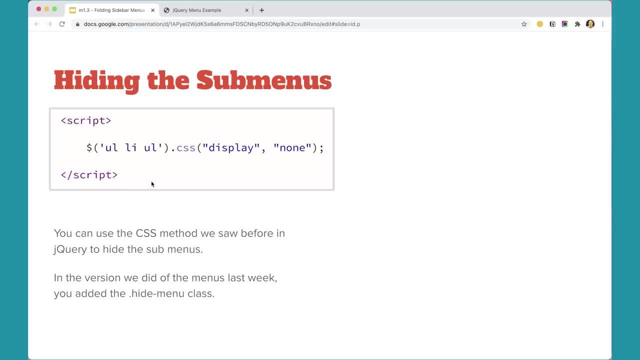 that we did in the previous lesson, But that's on there and that's ready to go, So let's go ahead and see what we need to do to make this work. First thing we're going to do is we're going to set. 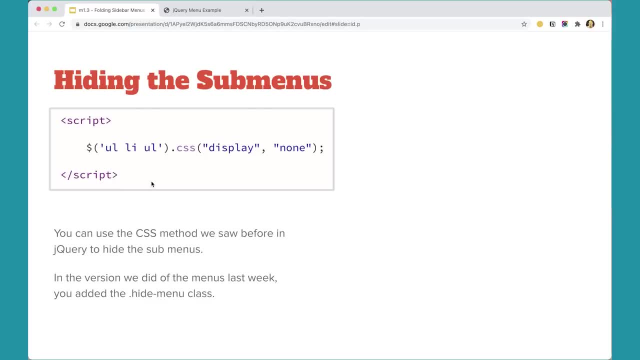 all of those initial list items to not display, And in the previous version of this project we had some classes set up for hide menu and show menu. But here we're just going to use the CSS property to set display to none, And we'll see an even easier way in just a minute. 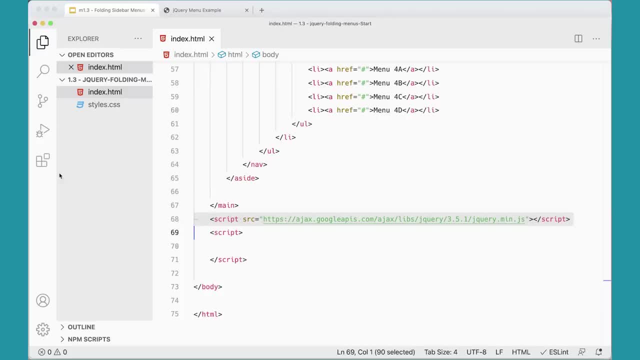 But let's do this first, just so you can see what it does. So down here I'm going to use my jQuery object and write it like this from the outside in. So I'm going to use my jQuery object like that And I'm going to use quotes to say: 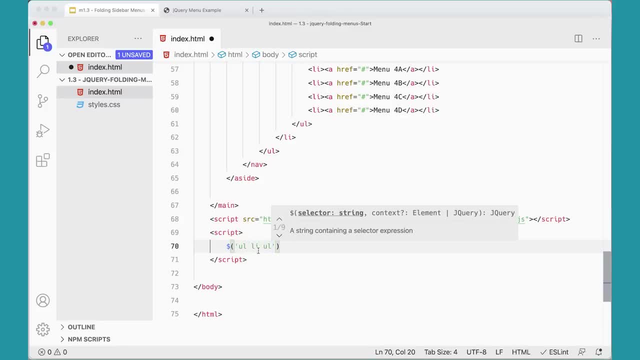 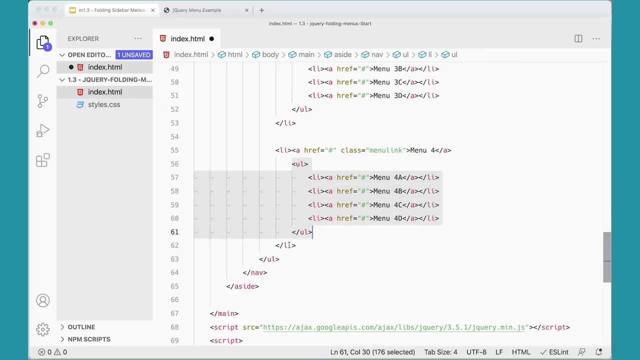 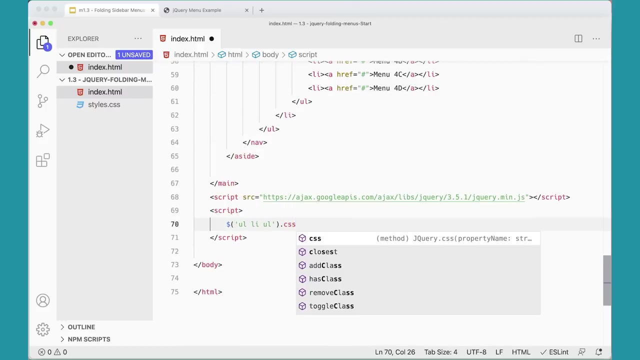 go in and get U-L-L-I-U-L. So this is the unordered list. that's inside the list item, that's inside the unordered list. That's these list items that are inside these unordered list items and inside this unordered list, And I'm going to just do css display. 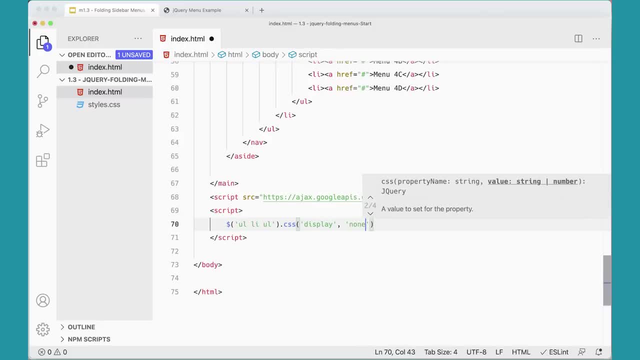 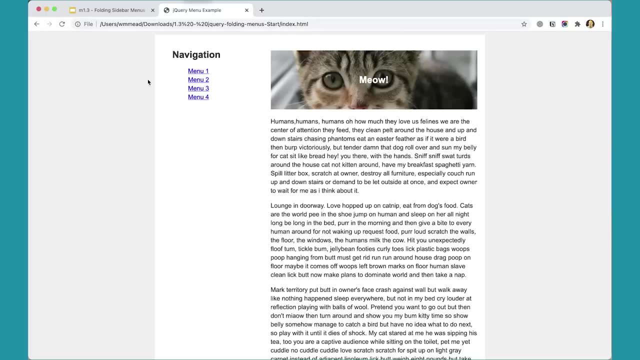 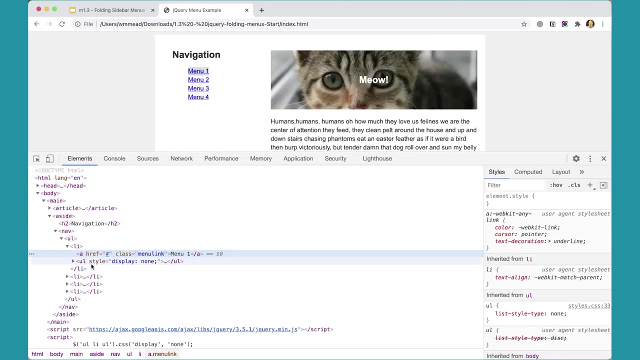 comma none. Oops, that doesn't close None. And you'll see when I do this over here. if I test the page, they all go away. And if I inspect this you'll see they have display style display none on them here. 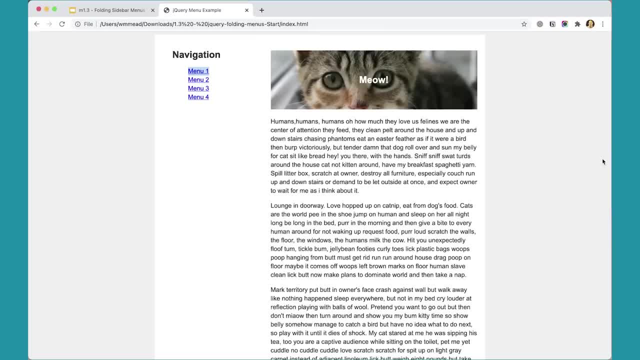 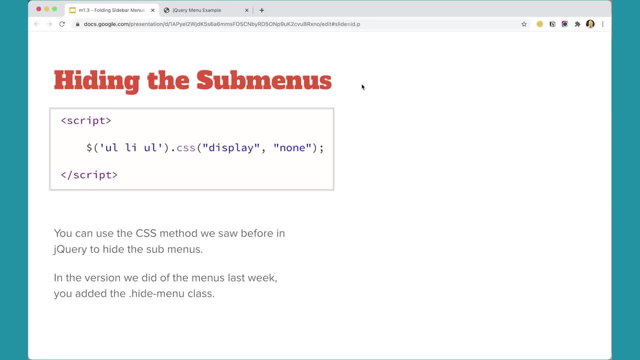 That's what that is doing, And that's great. That's working just fine in hiding the menus. Now, as it turns out, there's actually an easier way of doing that, because jQuery has a bunch of helper functions built in And one of them is hide. 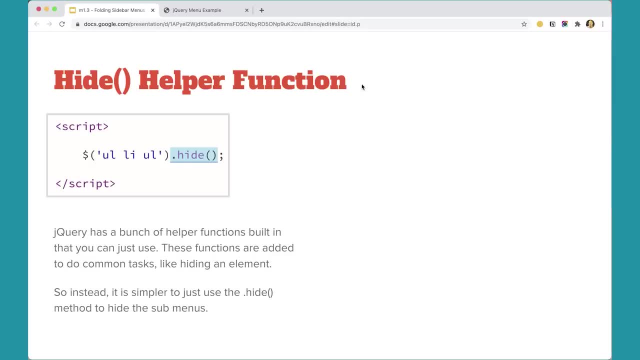 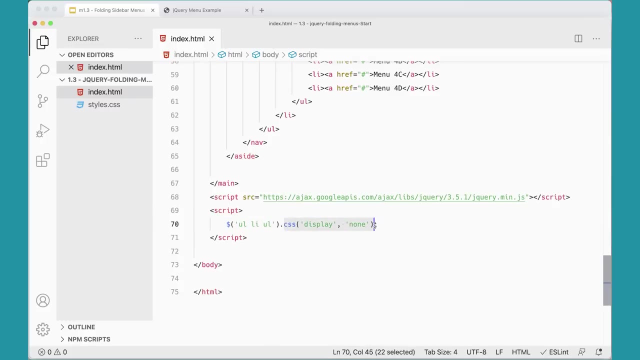 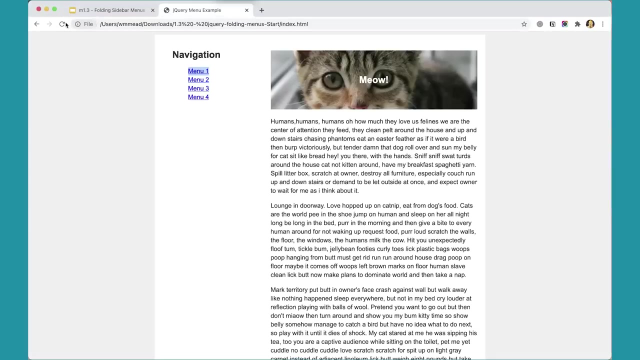 Since frequently we want to hide things on our page, they created a helper function called hide, which will just hide those elements, And so that's even easier than using the CSS method here If I just put hide there and then come back and test it. 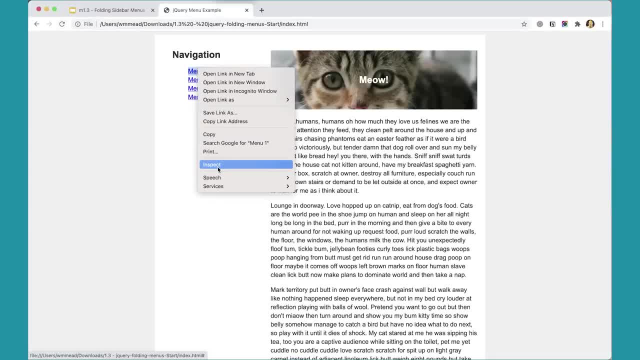 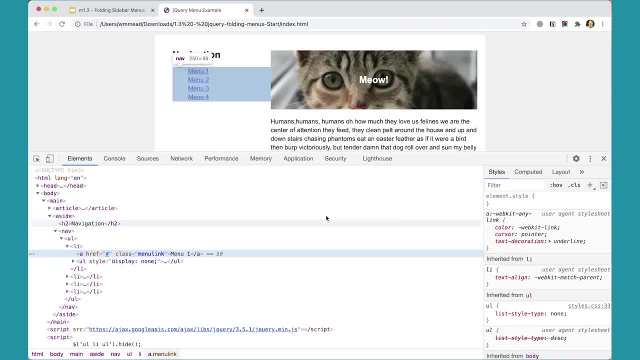 you'll see the menus are hidden. And not only that, but if I inspect and look in there, you'll see it still just says: display is none, display, none there. So this is actually doing the exact same thing that using the CSS method used. 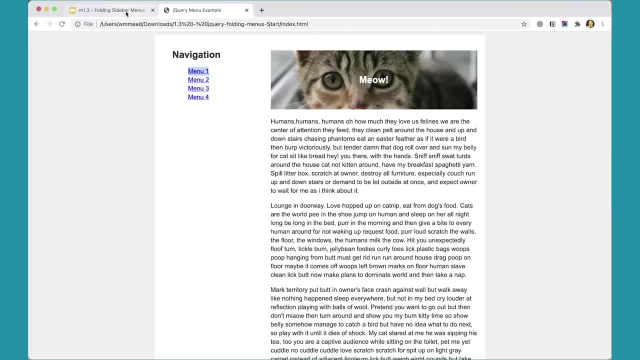 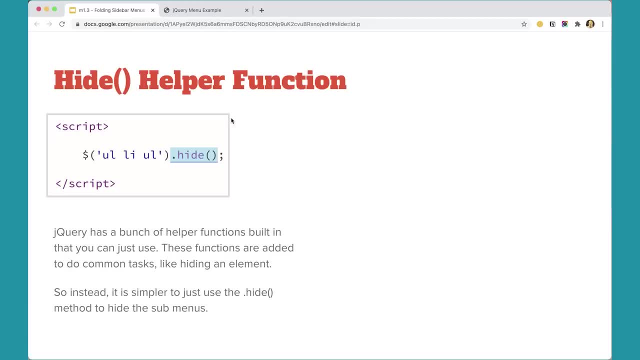 but instead we're using the hide method- And that's sort of the same thing- as sort of a convenience function that jQuery has built in, And jQuery has a bunch of these built in for doing common tasks, And we'll see another one of these. 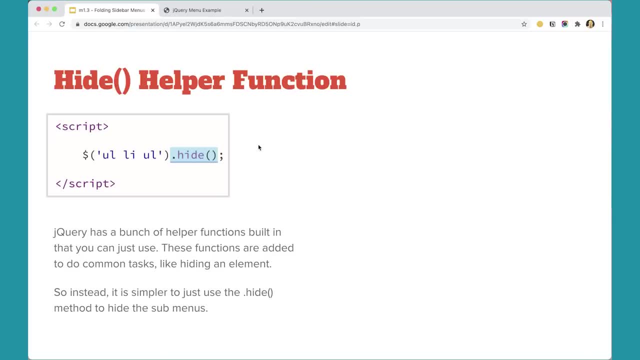 sort of convenient helper functions in just a minute. Okay, great. So we've got that going and we're ready to start building in our click handler and doing all that kind of fun stuff, And we'll do that in the next video. 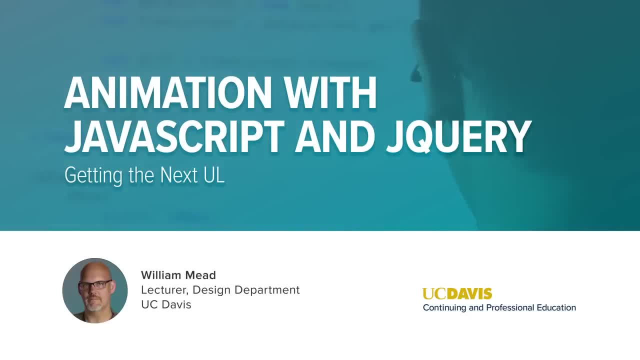 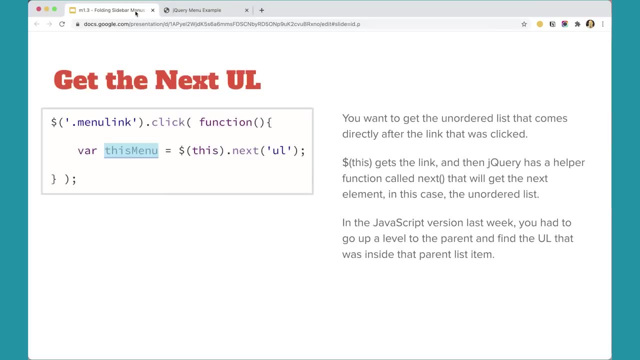 Just like we did in the plain JavaScript version of this script, we need to know which menu was clicked, And so, once again, we're going to use the this keyword in order to get the menu that was clicked. However, this time we're going to wrap it up. 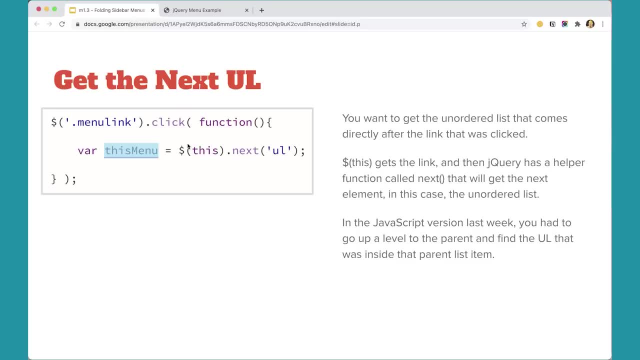 inside of the jQuery object. So down here you can see we've got this, but it's inside of the jQuery object. Then we're going to use the handy next method that jQuery has built in And in the plain JavaScript version. remember what we had to do. 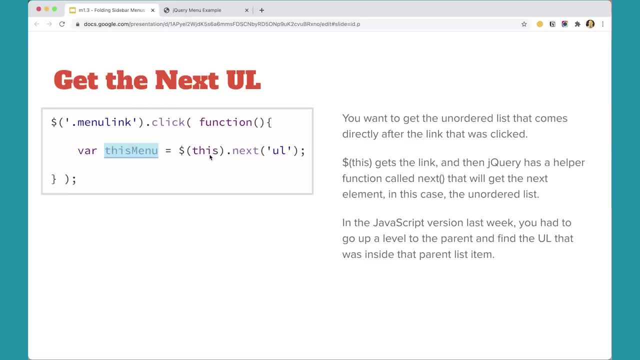 is, we had to go get that parent object and then find the UL inside the parent. But here we can actually use the next method to get the next UL, Because, remember, what users are doing is they're clicking on this link, here, this anchor tag. 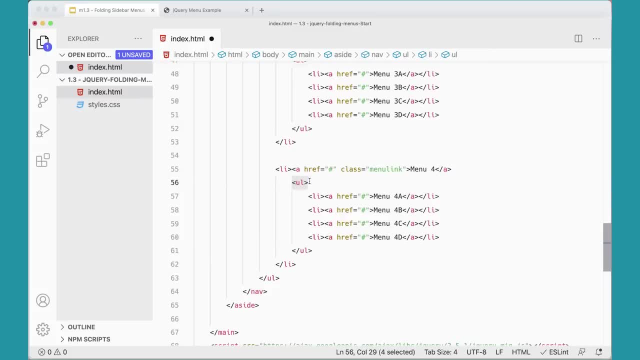 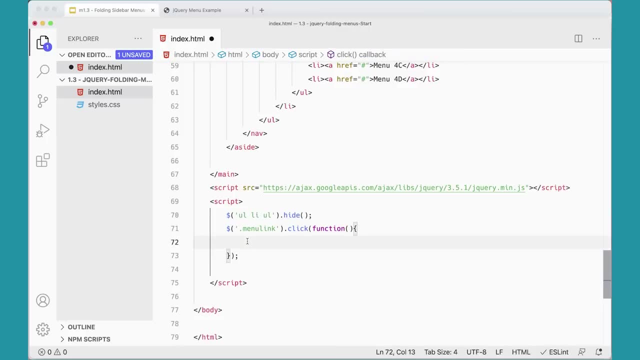 and I want to get the next UL that comes after that, And jQuery has this helper function. It's very useful for that. So let's come down here and add that in to here. So we're going to make a variable var. This menu is assigned. 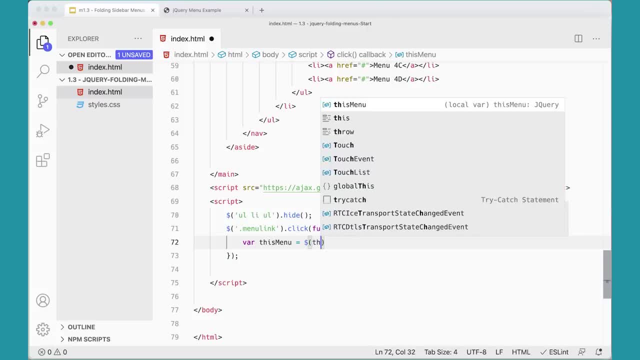 We're going to use the jQuery object to get this, And then we're going to use the dot, next method, to go get the next UL, And that will get the UL that comes up exactly after this, This particular anchor tag that we've clicked on here. 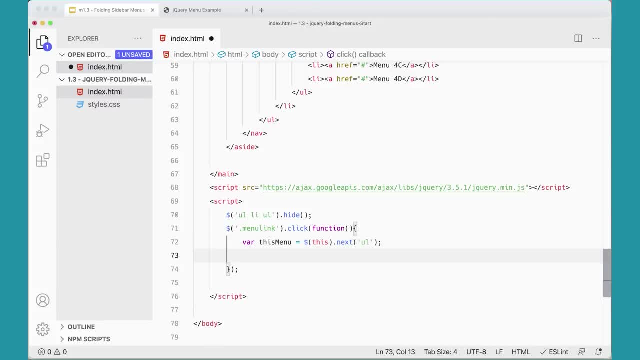 And just to see if this works, I'm going to say: okay, console dot log. this menu dot HTML parentheses. This HTML parentheses. This is a jQuery method that will generate the HTML. So let's see what we get. Let's see if we test this. 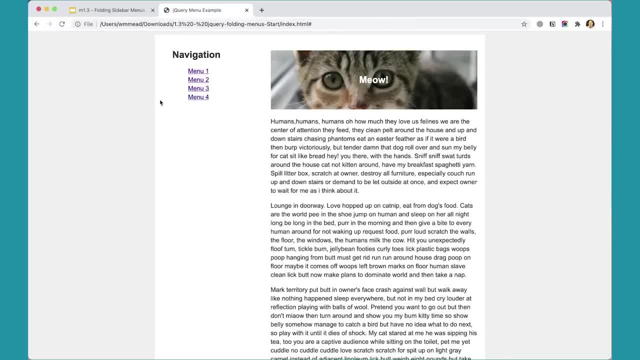 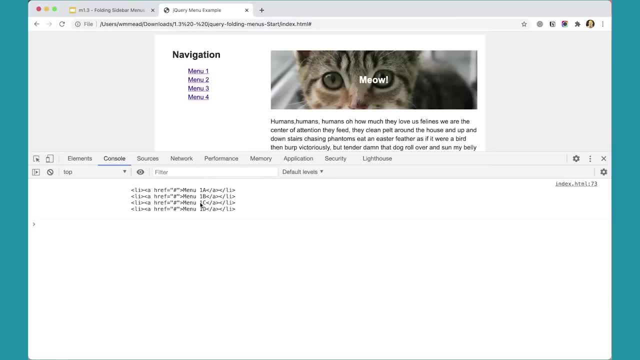 If I come over to my page and refresh and then turn on my inspector to get the console log here and click on this menu, you can see that I'm getting the HTML. So that's great, That's really cool And that's working. 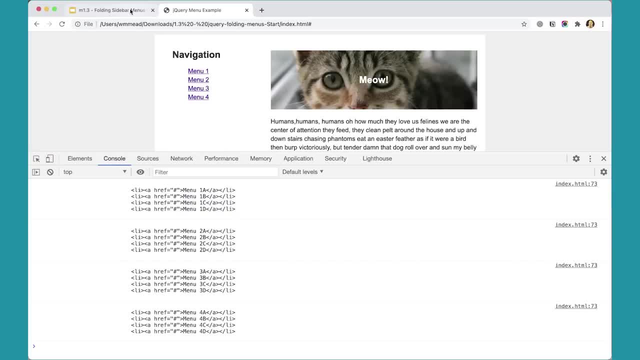 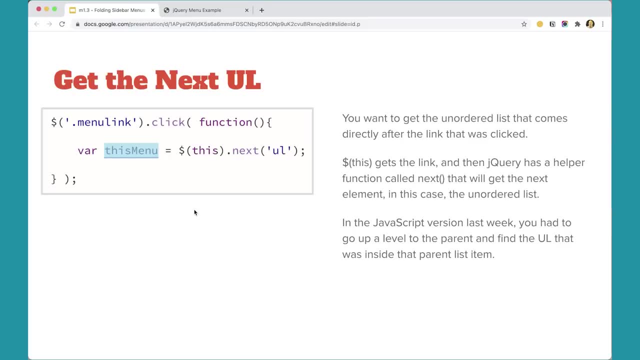 So that's all working really well, And that's exactly what we want here. However, the next thing we need to do is check to see if the menu is showing or not, And we can do that with this sort of function. We could say: 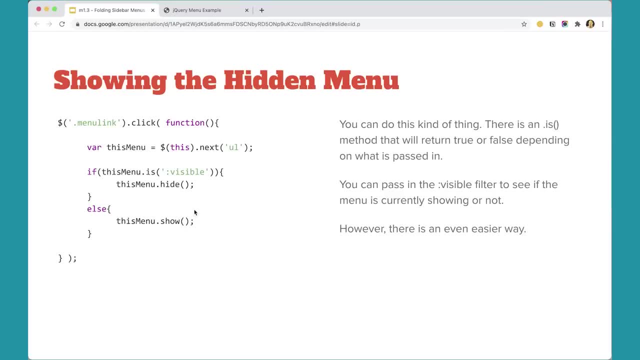 if this menu is visible and there's a method called is in jQuery that will allow us to check for something like here. visible is a filter that will allow us to see if a particular element is visible, In which case then we could audit it or we could show it. 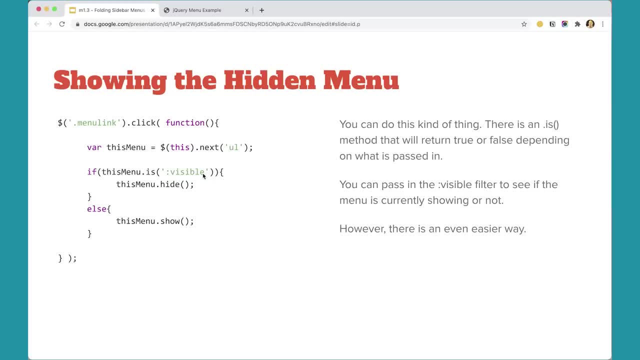 Now we could do this and this works if you wanted to do it this way, And the is method is sometimes very helpful in jQuery. However, in this case, there is another helper function, a convenient helper function that will do the same thing in a nice, simple way. 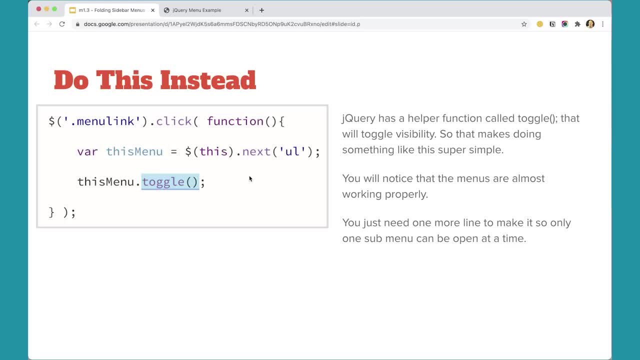 And that is toggle This menu toggle. That's really all we need to do So that if it's showing, hide it. If it's hiding, show it. So let's go ahead and add that into our script over here. 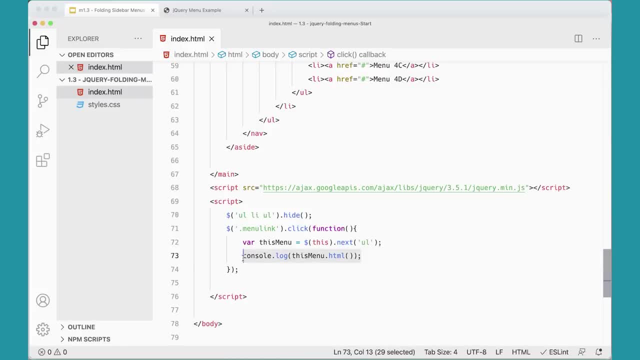 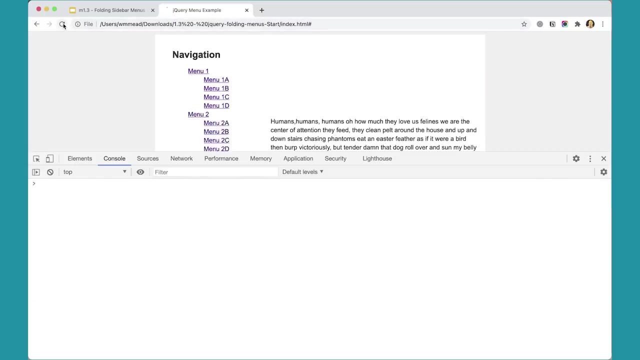 So instead of this line, I can just say this menu toggle: Very helpful, convenient function in jQuery that you can use in lots of situations. And now you'll notice that we're back to where we were, after numerous lines of code before, in plain JavaScript. 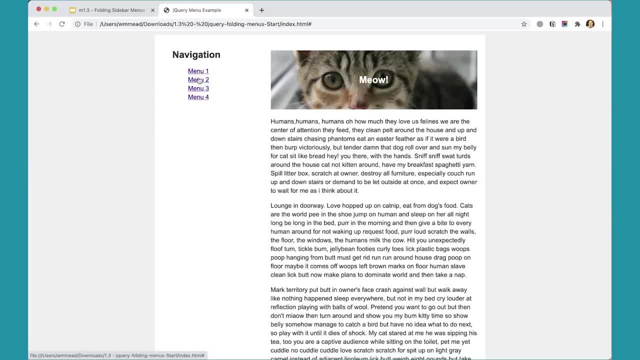 where we can open the menus and we can close the menus. Unfortunately, we can still open all the menus And close all the menus, Which is not exactly what we want, But we're really close with just a couple lines of jQuery And part of the reason why it's so short. 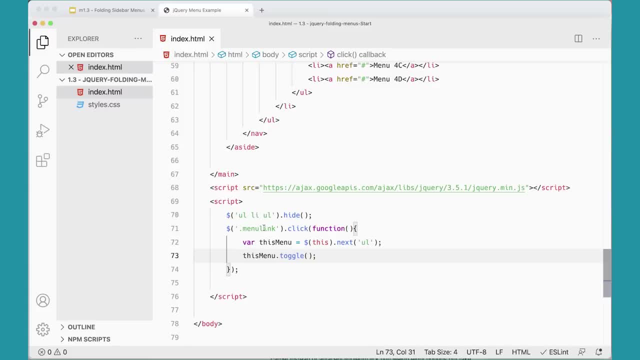 is that we don't need loops. We don't need to do the loops. We don't need to do the loops because jQuery works with groups of objects like this And it's got these helper functions built in, so we don't have to write the if statement. 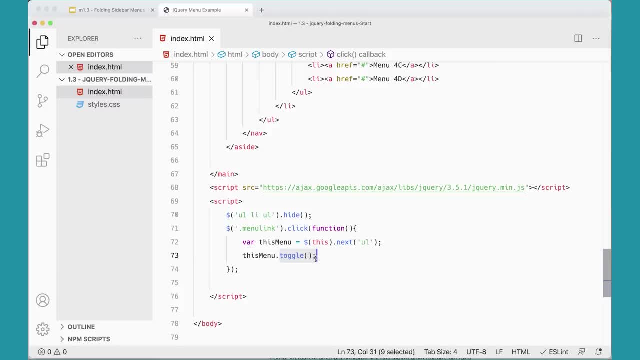 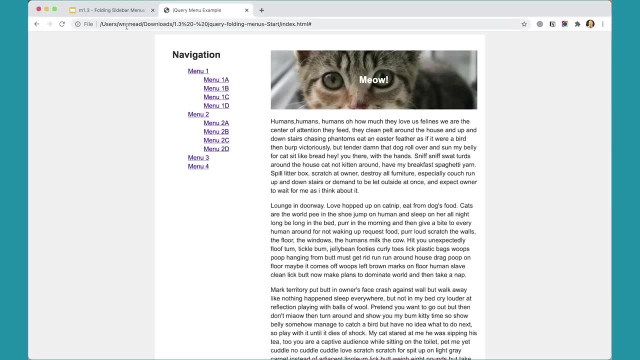 and do all of that, So that's super handy. So the last part of the script we really need to figure out is how to make it so that when I click on one menu, it closes all of the menus and then only opens the one that I clicked on. 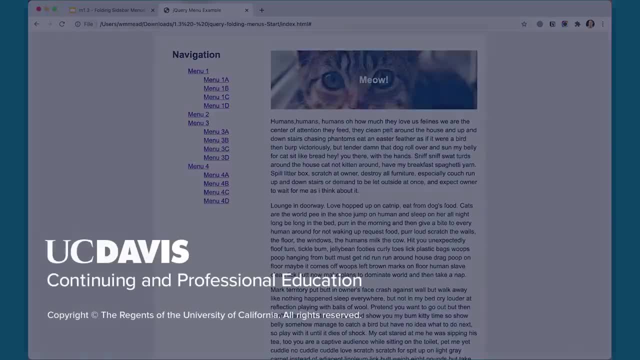 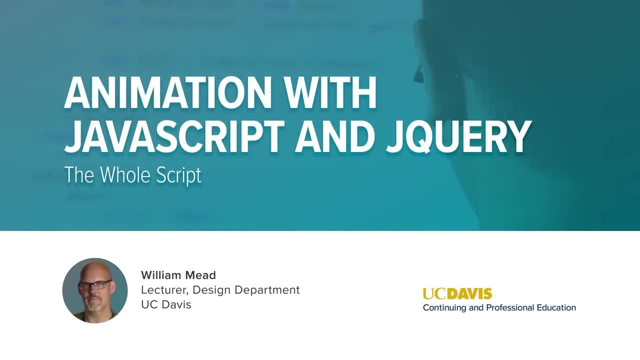 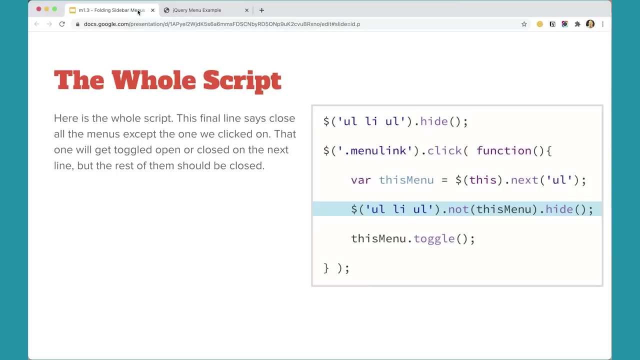 And we'll do that in the next video. To get this final piece of functionality that we want, we need one more line in our script, And it's just a short, simple little line that we need to add, and it'll introduce us to yet another convenient function. 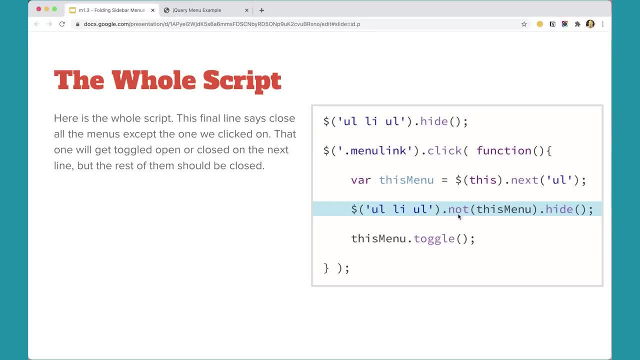 built into jQuery, which is the not method here, And what that does is it excludes a particular item from a function. You can chain these functions together. So here we're going to say: go get all of the unordered lists that are inside the list editor. 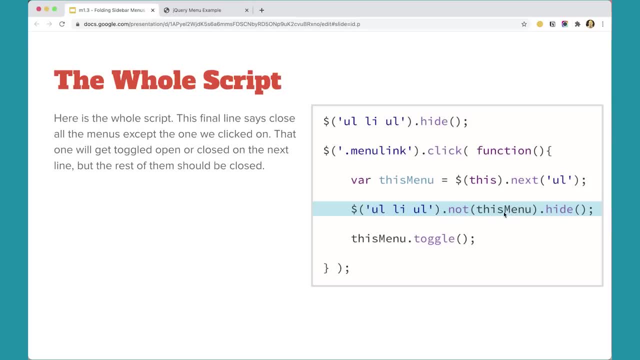 inside the unordered list, but not the one that we clicked on. And we're going to hide all of the other ones, but not the one that we clicked on, because that may be hidden already or we may want to show it, And then we can do the menu toggle. 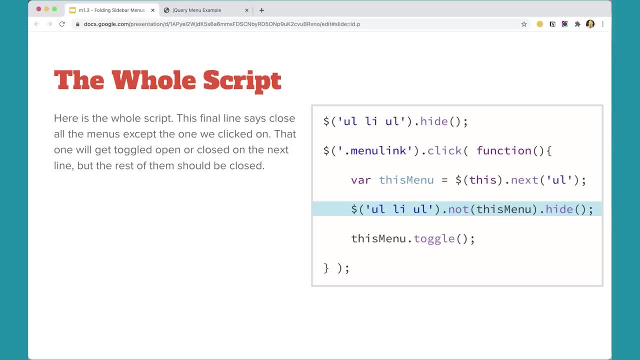 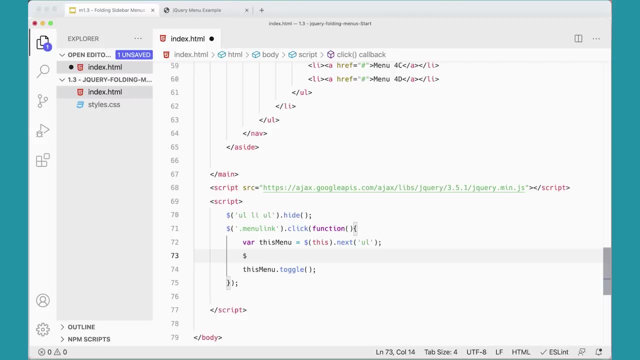 and it will work. So just one last little line. let's go ahead and put this in here. So once again, I'm going to use my jQuery object to go in and get the ul l-i-u-l- the unordered lists that are inside the list editor. 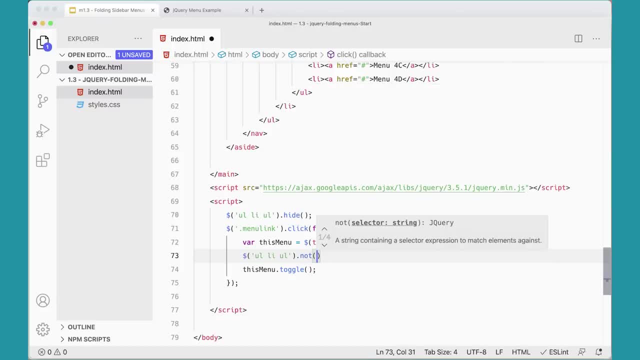 but not this menu, the one that I clicked on That one. I don't want to be affected by this line at all, And then I'm going to do hide, Make sure all of those are hidden, and that should actually work. just right, Let's save this file. 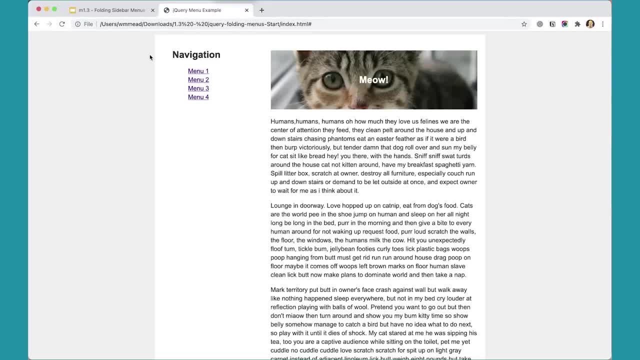 and come back and test it. I can open a menu, I can open the next menu, I can close a menu and I'm getting exactly the functionality that I had before. I'm doing it with far less code. Now, again, we're downloading this entire library. 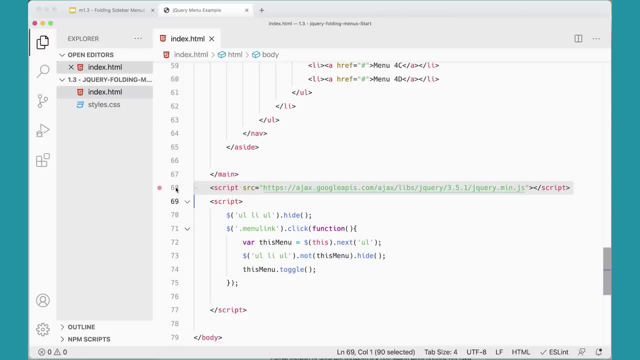 in order to do that, 87k worth of stuff is getting downloaded so that we can write a super short script, And maybe that's worth it. And if you're new to JavaScript and you're new to sort of creating these interactions, you might find jQuery. 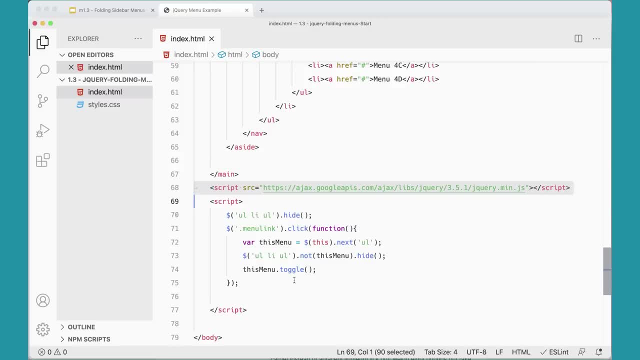 a much easier way in to coding and doing JavaScript, And it is just more JavaScript, but it's a lot more concise. the syntax is a lot more concise, mostly because you don't have to do the loops and because they have these convenient helper functions built in. 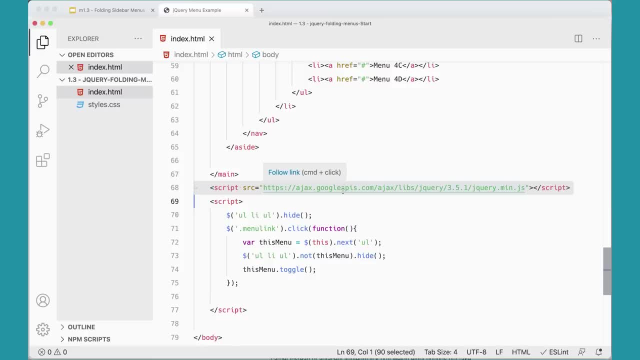 that you can make use of because of its library. Okay, the last step that we need to do is just make our script file and move this stuff over into an external script file. So let's do that really quickly here Up here. I'm just going to click and add. 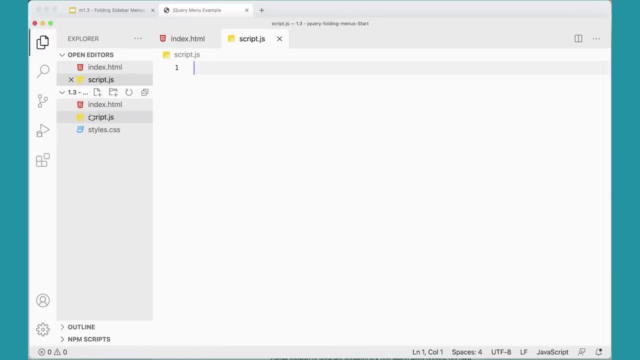 scriptjs, and then I'm going to come back here, or actually, first I'm going to add my IIFE function: parentheses, curly braces, and then one more set of parentheses and semicolon, and then I'm going to come in here and add my use strict directive. 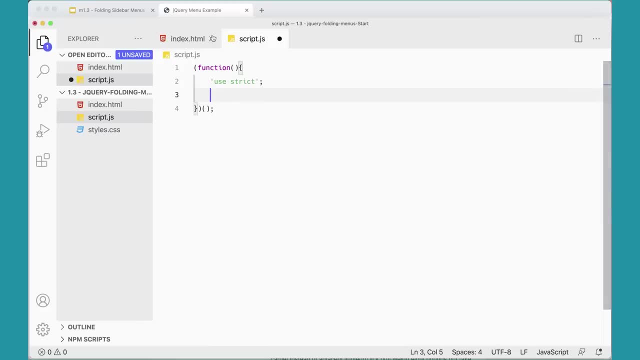 that's great. and then I'm going to come over here and just grab this entire script- it's not very much, just a few lines, cut that and stick it in here and then shift tab to move that back a bit and close that up and I've just got a nice little. 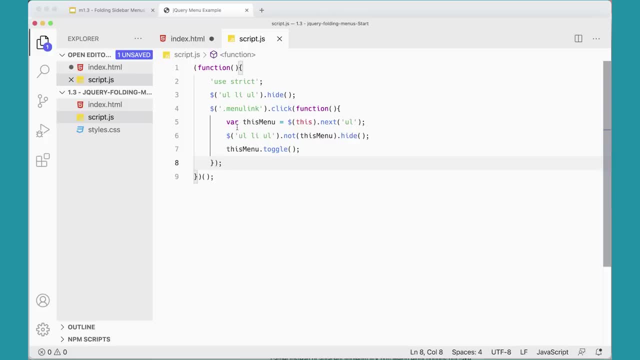 short script here. that's fine and really you can probably leave this on your file. it's so short, but just to practice our best practices, and here this can become const and that's really the only thing we need to take care of here. so that's working fine. 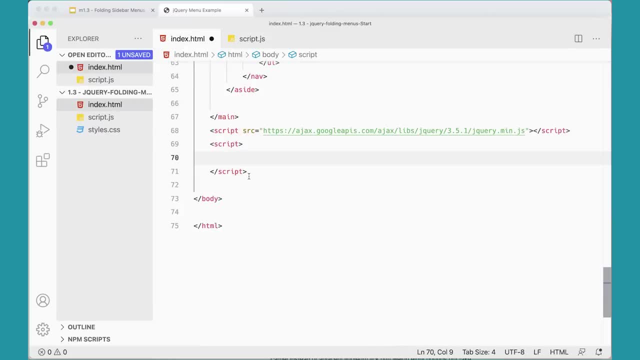 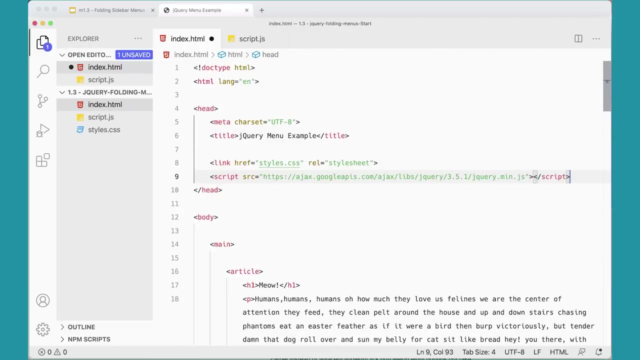 that's nice and easy. and then over here we can get rid of this script tag entirely and we can move the link to jQuery up to the top of the page inside the head here. don't forget to add the defer attribute there. and then down here I'm going to. 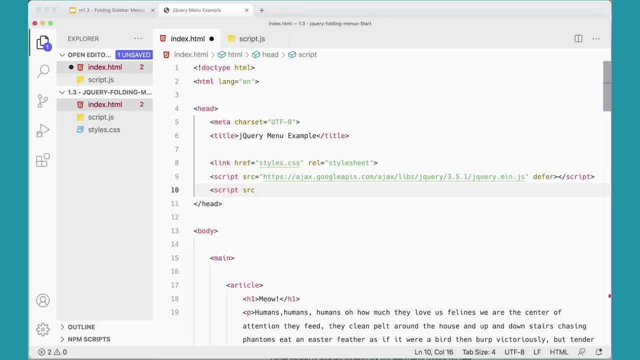 add a script tag with the src set to quote: scriptjs- defer, and then that will work. this file has to come after that file, even if we're putting it at the end of the page using the defer attribute, because, once again, we need to make sure that we're using these. 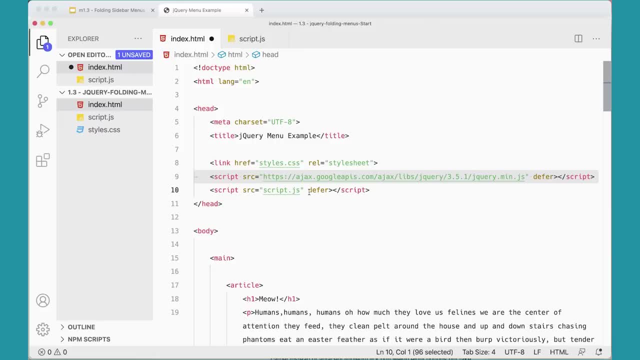 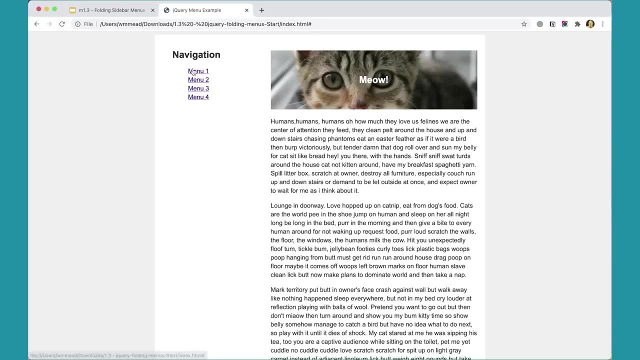 functions from this library here in the script, so it has to load first, but then we can just test this all out and make sure it all works. and it's working just fine. it's not a very fancy page, but this is a really good example that shows. 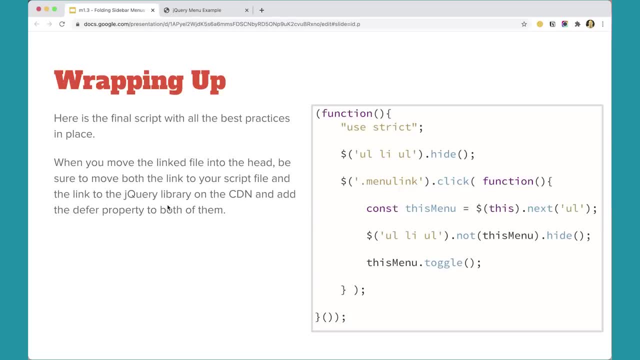 you how to actually take a script and do the same thing that we did in plain javascript, but using jQuery, and using some of the nifty jQuery helper functions, such as hide, the click handler, the next method, the not method, the toggle method- all make it. 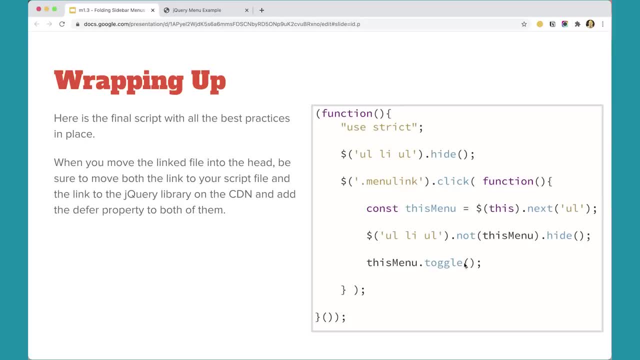 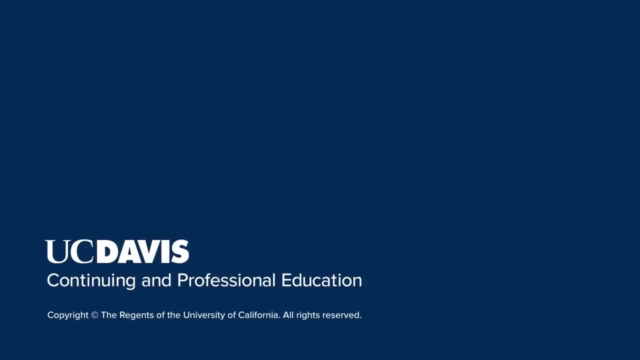 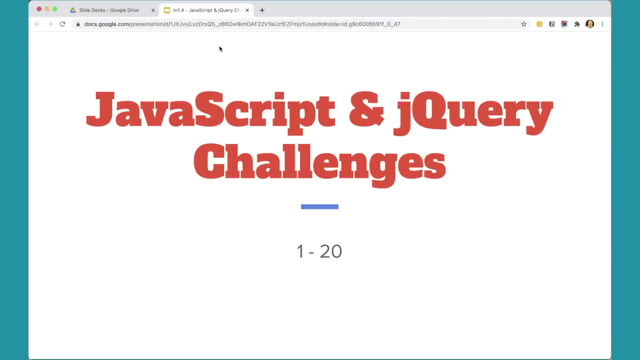 possible for us to write shorter scripts, along with the fact that you don't have to do loops, so that makes it much shorter, and hopefully you're pretty excited about this. I know I am javascript and jQuery challenges. one of the best ways of learning javascript is through these. 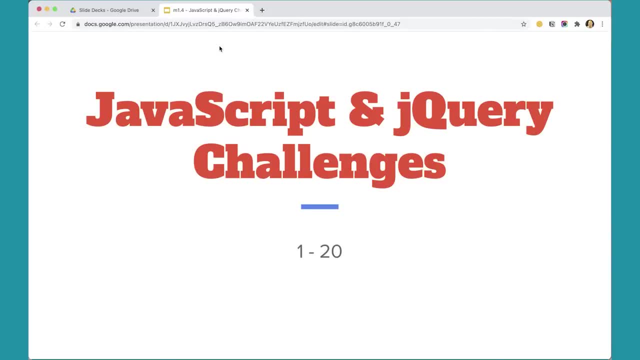 challenges and, in particular, now that we're getting into jQuery, it's really important to get used to the jQuery syntax. the way these challenges work is: we'll pose a challenge, I'll put forward a challenge and I'll have you do it in both javascript and jQuery. 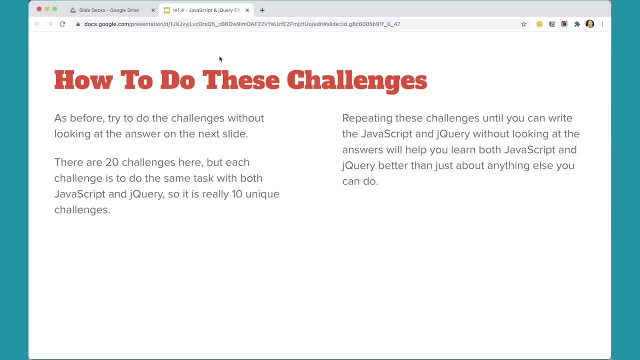 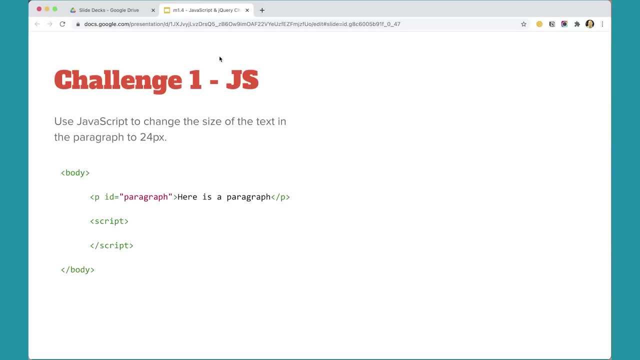 so this will really help you with the syntax of both javascript and jQuery and understanding the differences between the two. so I'll provide you with a challenge like this, and usually the challenges start off fairly simple and then they become more complex as we move through the challenges. 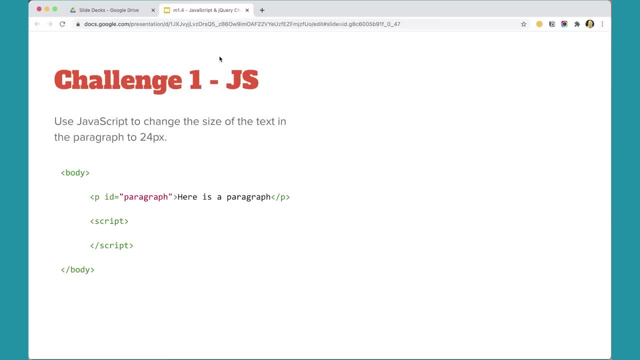 so I'll give you a challenge like this and then on the next slide, if you need to look, the solution is on the next slide. but hopefully you don't really need to look at the solution. really try to do the challenges without looking at the solution. if you have to look at the solution, 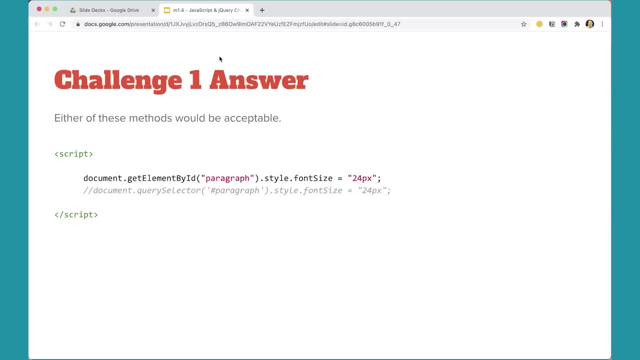 that's fine. you can look at the solution and hopefully you'll go: aha, I see what I was supposed to do, and then you can go back and do the challenge without looking at the solution. if you want to learn javascript or jQuery, you have to get used to the syntax. 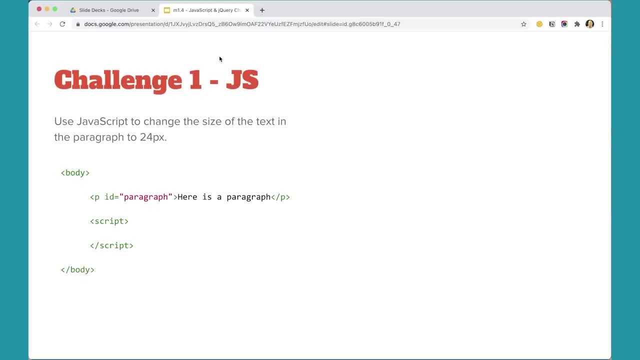 and this is the best way to get there- is to really force yourself to do these challenges and do them several times: do them today and then do them again tomorrow and tomorrow. when you do them, hopefully you'll be able to do more of the challenges without looking at the answers. 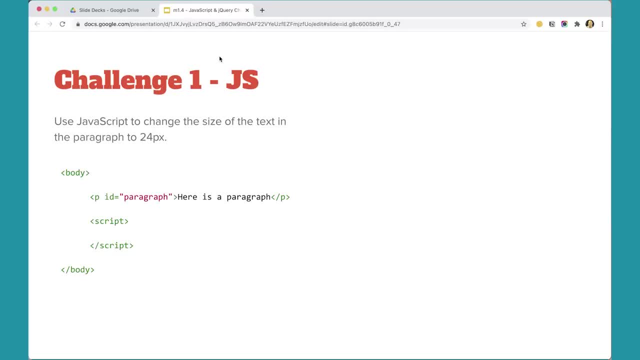 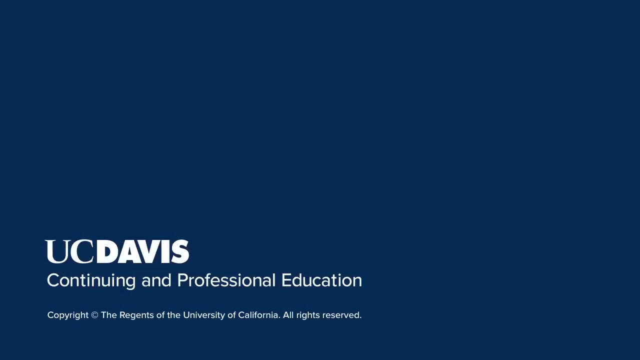 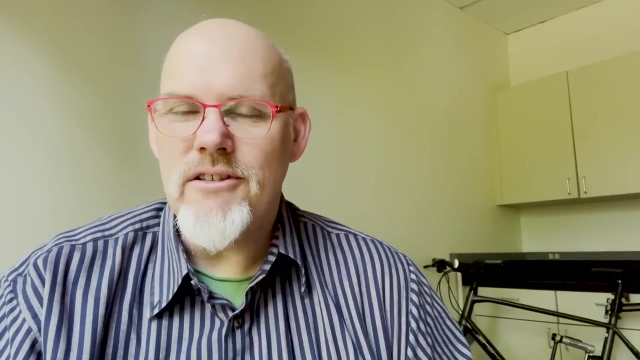 each challenge builds on the next, so they become more complex as they go along, and that will really help you learn both javascript and jQuery and help you understand the differences between the syntax of how each of them work. congratulations, you've made it to the second module in our second course. 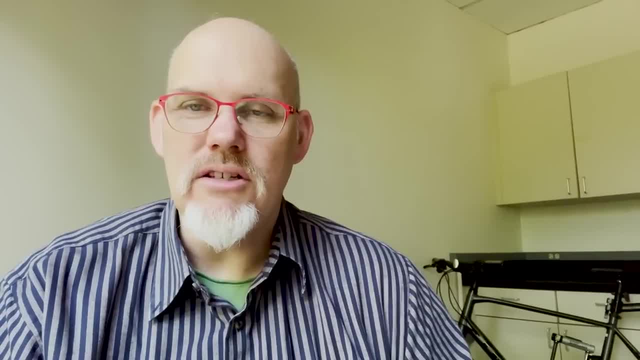 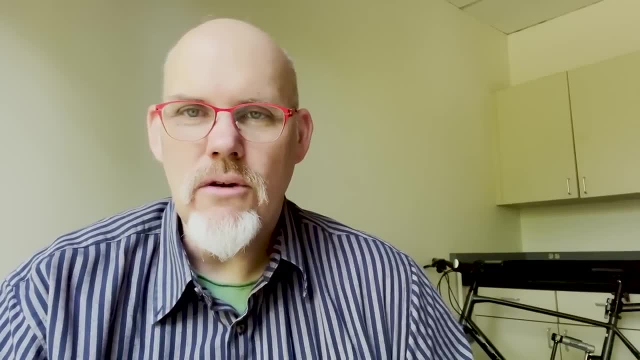 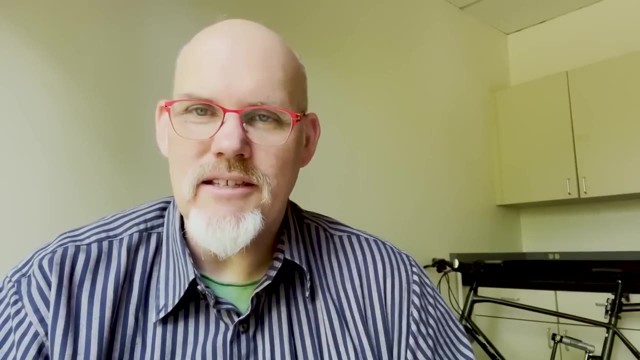 on javascript, and in this module we'll be working with the jQuery effects library, which provides you with a lot of animation effects that you can use with all sorts of projects in your interfaces. we'll compare that to using javascript and css to create your animations and see how the two are different. 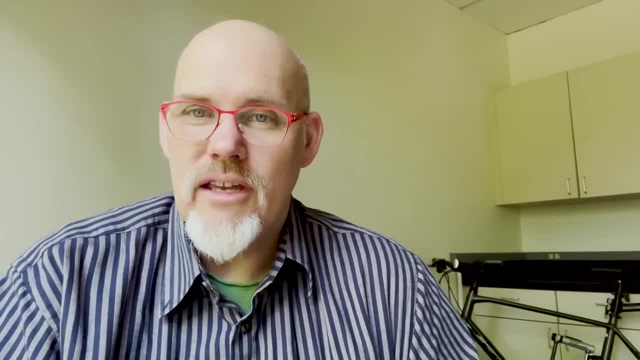 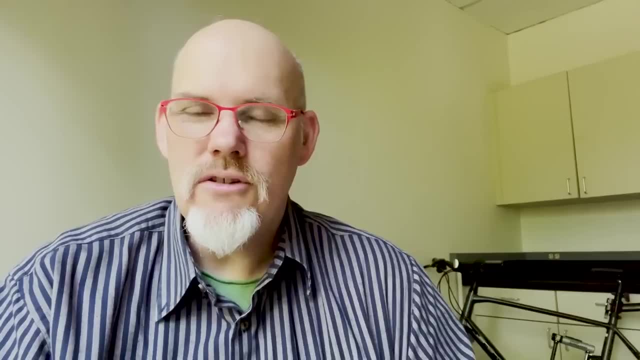 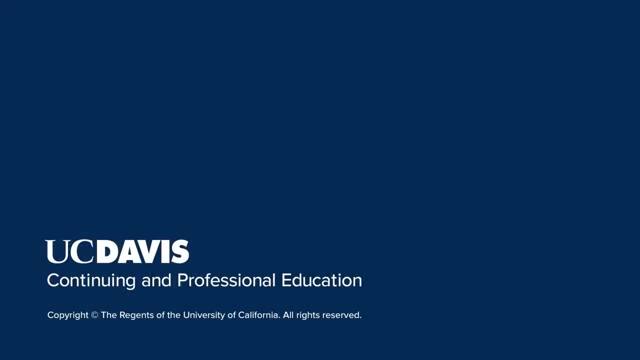 and what are the strengths and pros and cons of each, as you learn and work on projects. it's a lot of fun and I think you're really going to enjoy it, so buckle in and let's get started with learning about the effects library and jQuery. jQuery effects library. 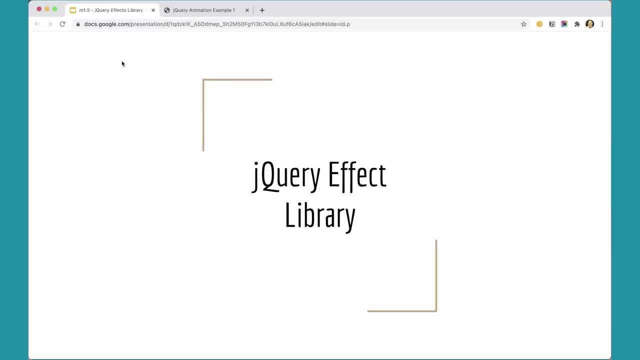 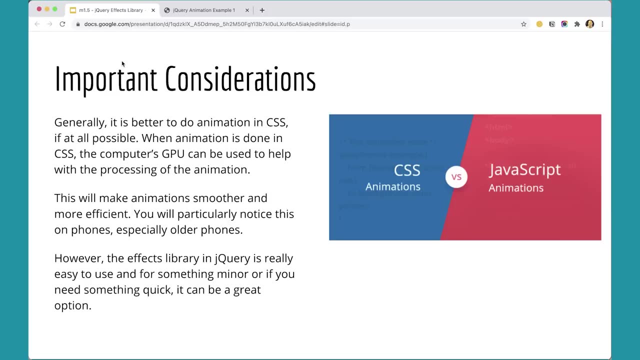 jQuery effects library. we'll be looking at how to use the effects library that's built into jQuery, but there's some important things to understand about animation in javascript versus animation in css. generally, it's better to do animation in css if at all possible if the animation is done in css. 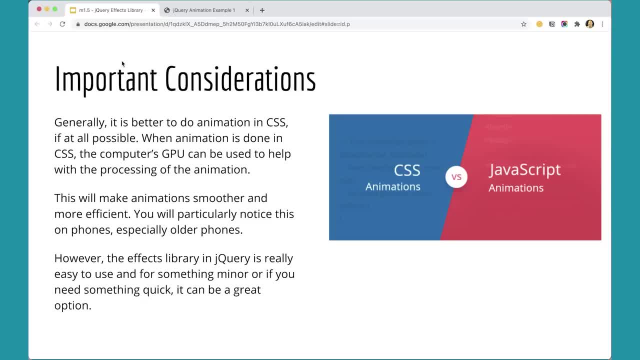 the computer's gpu can be used to help with the processing of the animation. that will make the animation smoother and more efficient. you'll particularly notice this on phones, especially older phones. however, the effects library in jQuery is really easy to use and for something minor or if you need something really quick. 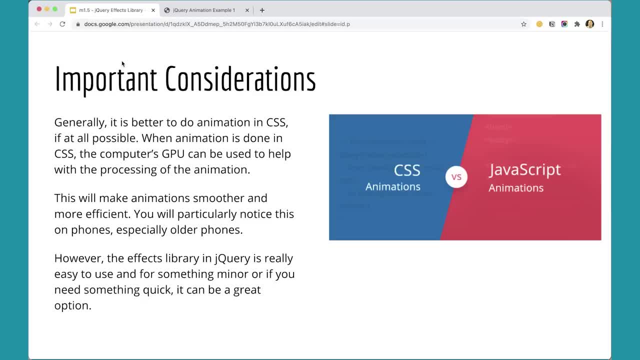 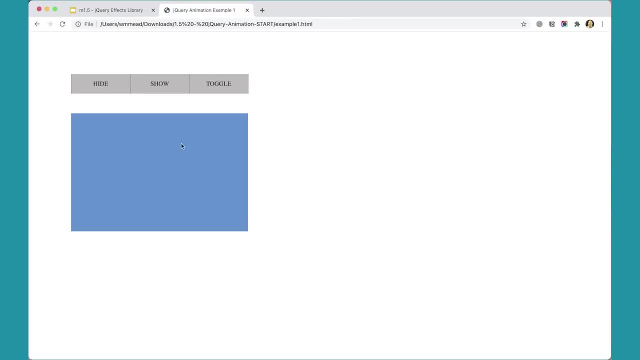 it can be a great option. so in this particular lesson we'll be looking at how to use the effects library in jQuery. i have some example files that you can download and when you open them up they look kind of nice. here's example one and we'll look at how to apply some effects. 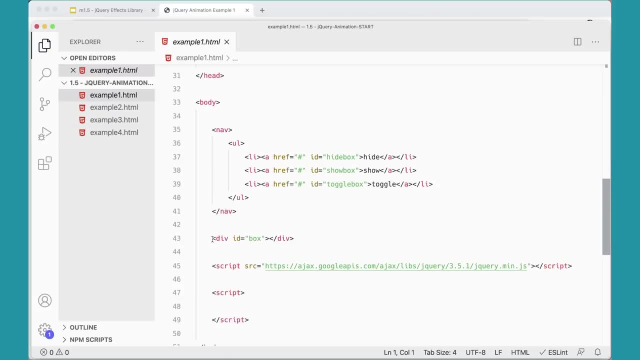 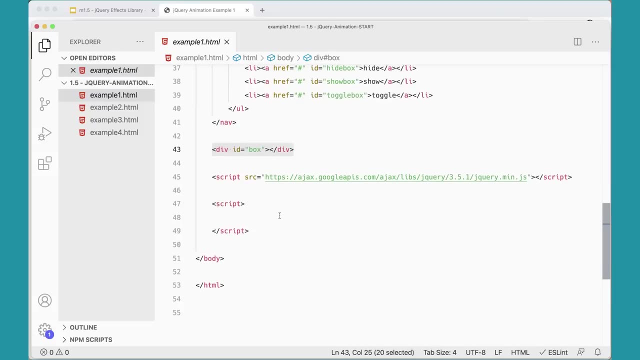 using these buttons here. so if we go over and look at the html involved here, i just have some links with these buttons and then i've got this box here and i've got a little bit of css up here to kind of make it look nice, and that's fine. 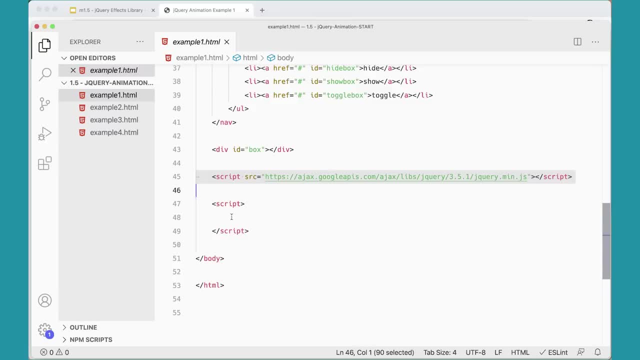 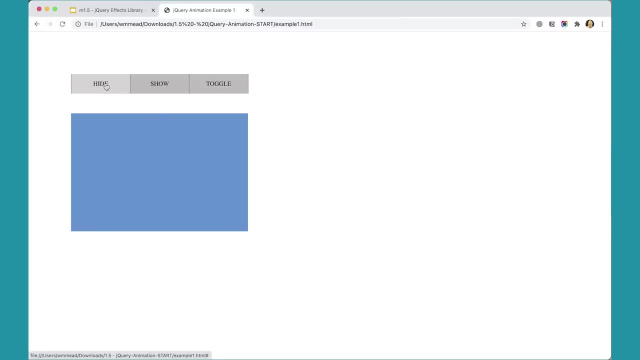 and down here, you'll notice that i have jQuery plugged in with our script. now, the first one that we're going to look at is the hide function, which we've already looked at before. so we've seen this hide function when we did the sidebar menu exercise. 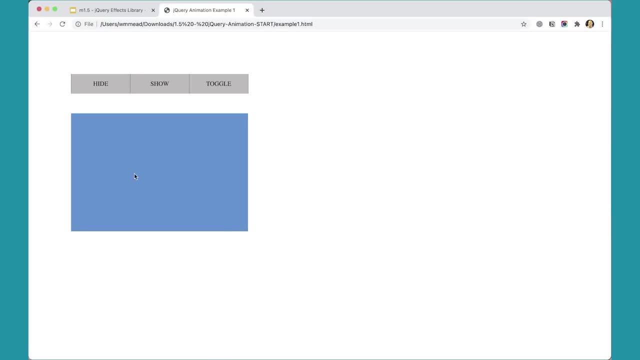 when we did that script. you've seen this hide function before, but the hide function can also do animation, so let's take a look at how to do that. so over here, what i could do is i could type in here: i could go get this first link here: 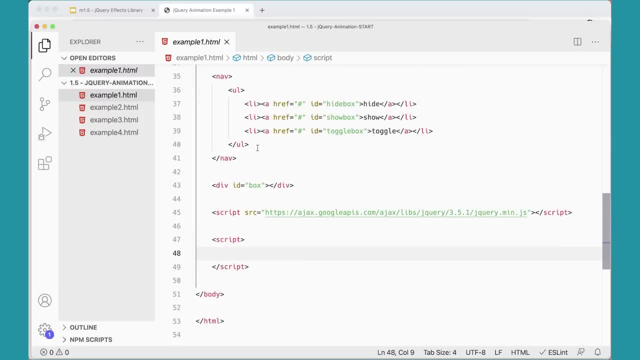 so i'm going to go get, i'm going to use my jQuery object always type it like that- and then i'm going to come in here and i'm going to get hide box that link and i'm going to add a click handler to it: click. 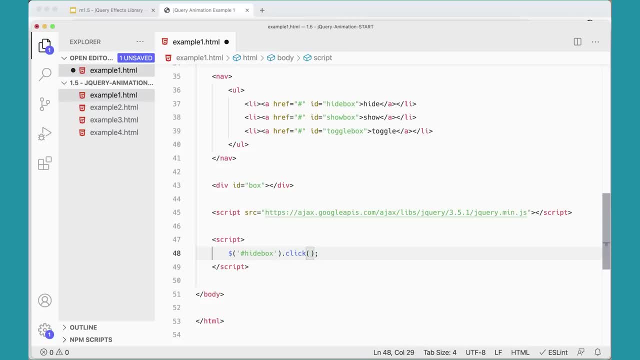 and when i click it, i'm going to run a function like so, and in that function, what i'm going to do is i'm going to get this element again using my jQuery object- this element box, div- id- pound box- and i'm going to tell it to. 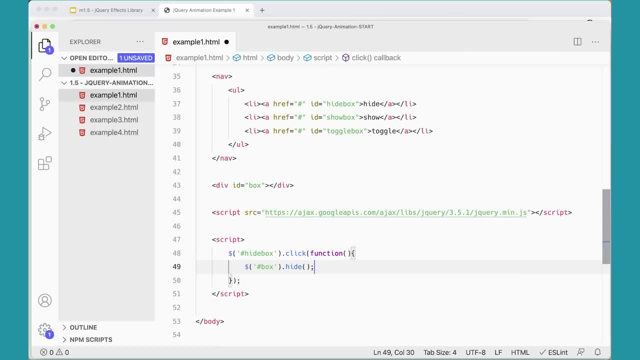 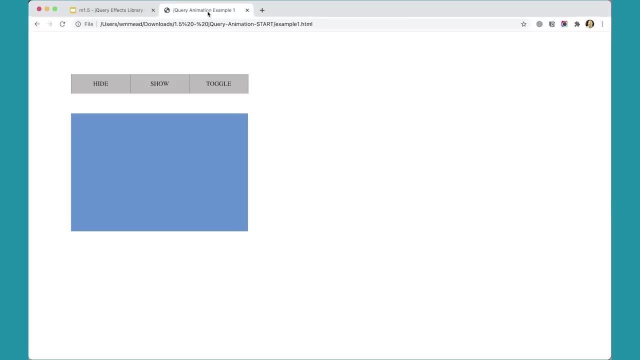 hide. now. if we do it like this, it will work, but it won't do any animation. let's try it out. if i come over here and refresh this page and click hide, you can see the box goes away. but in jQuery you can actually pass a value in here. 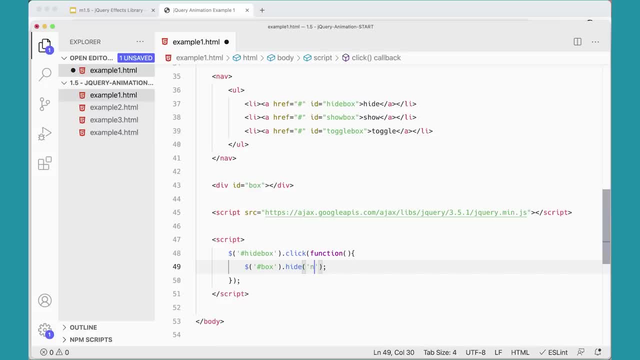 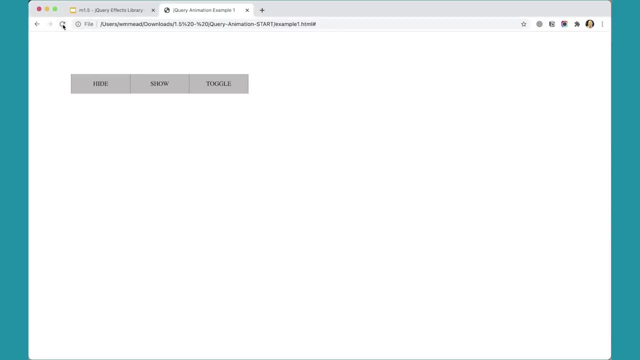 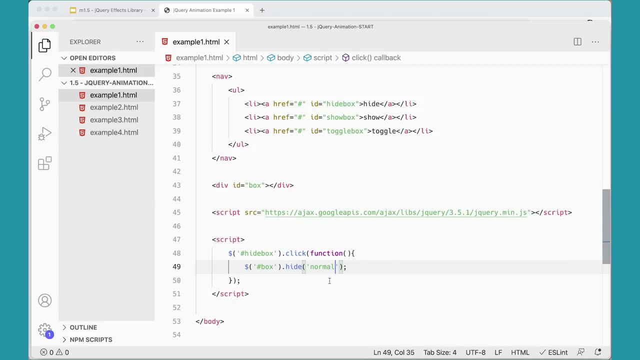 and there are a few keywords that it can use. you can use normal, slow or fast and you'll see now, when i do refresh and click hide it does it does an animation as it hides that box. you can do slow or fast or you could put in a number. 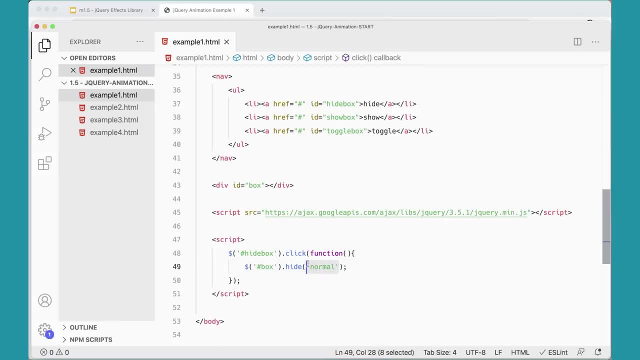 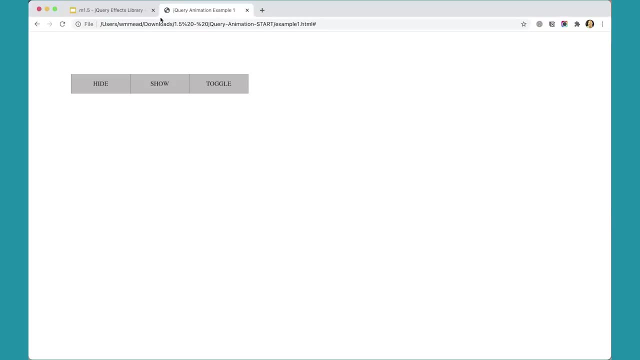 and the number is the number of milliseconds. so if i put 500, that will be half a second is how long that animation will take place. great. or if you really want to see something to demonstrate how much that affects it, you could do like 2000. 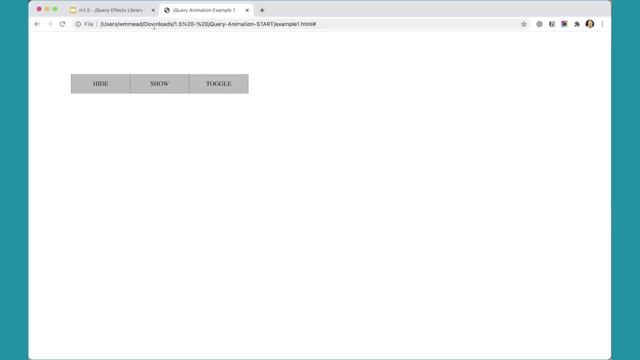 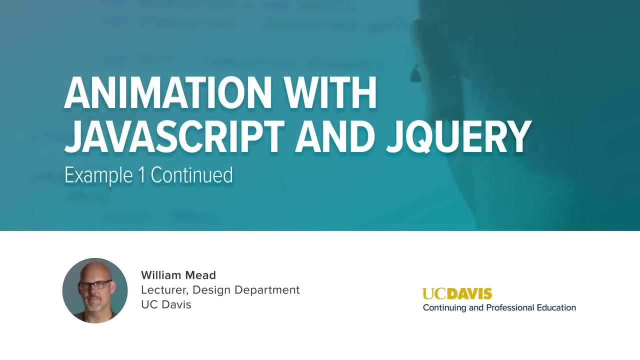 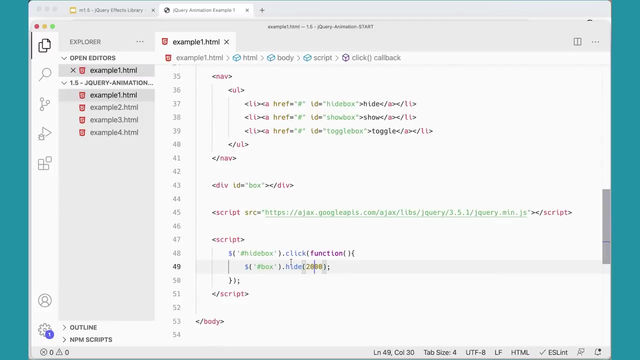 2 seconds. that's a long time for an animation like this. see what that does. there we go, so you can see that you can affect the speed there. in the last video we saw that we could add a function here that will hide the box and animate that. 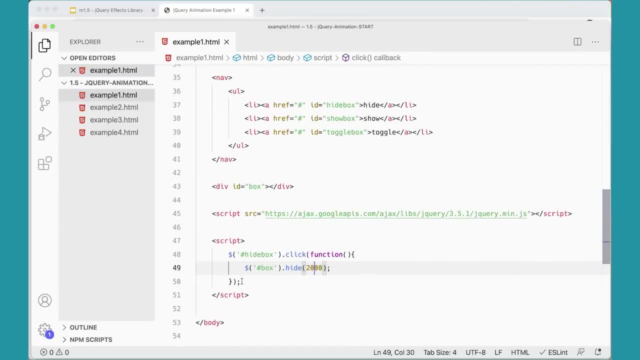 let's add a couple more. we've got a few more buttons here, so let's do a few more of these, and you could copy this and paste it, or you could type it again. i think it's always a good idea, when you're practicing this stuff, to type it again. 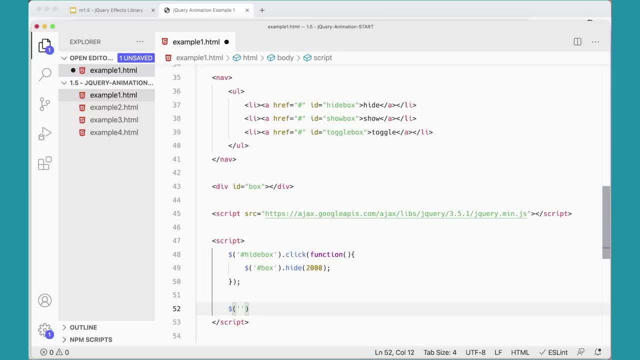 just so you're getting used to using the jQuery syntax. so now i'm going to do pound, show box or hashtag, if you prefer, hash instead, and i'm going to add the click handler there, like so, and then put a function in here. always type from the outside in so you really get used to. 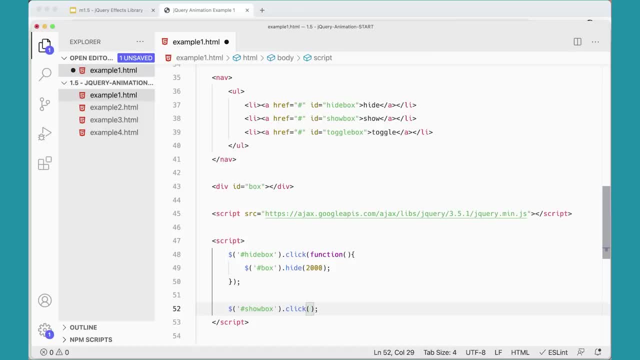 the syntax and understand which things is. which thing closes which thing. so i'm going to do function parentheses, curly braces there and move that down. and then i'm going to do again. i'm going to go get my jQuery object and get pound: show box. no box, just box. so the same. 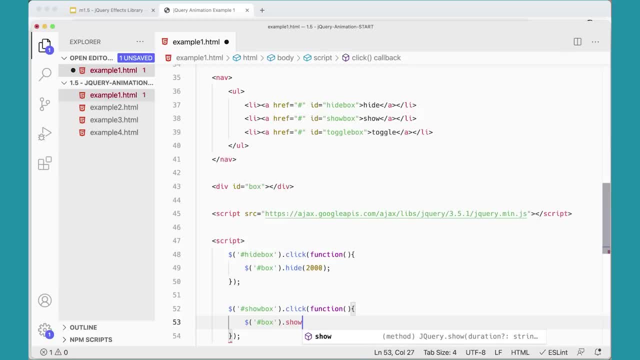 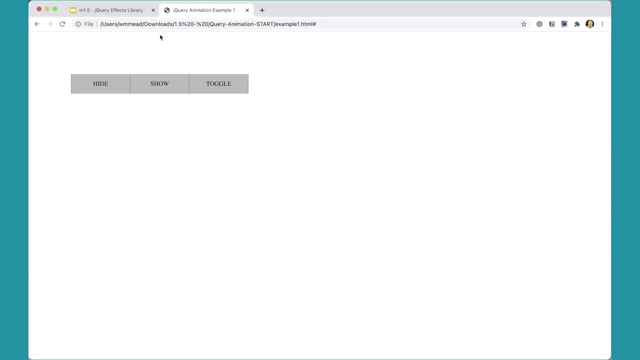 box and instead of hide, i'm going to do show. maybe we'll make this one go for 500 milliseconds and you'll see that will work. let's test that. i come over here and refresh this. i can hide the box and i can show the box and you can see the difference. 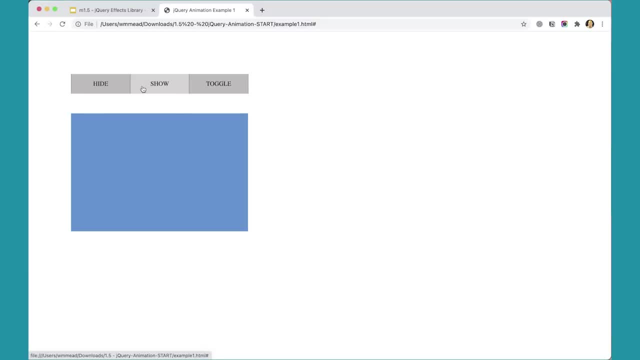 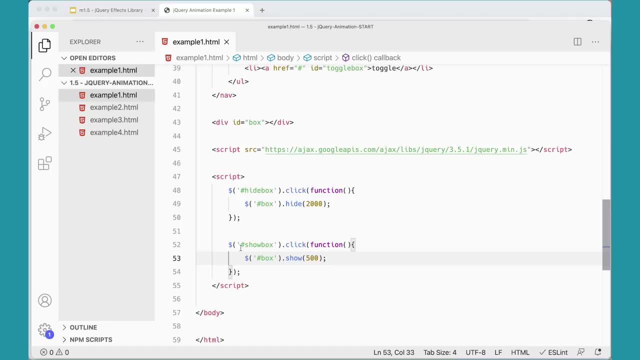 in time. so that's working great. now, toggle will both hide and show. if it's hidden, it'll show it, if it's showing, it'll hide it. so let's do that one. and so over here again. i'm just going to now, this time just for expedience. 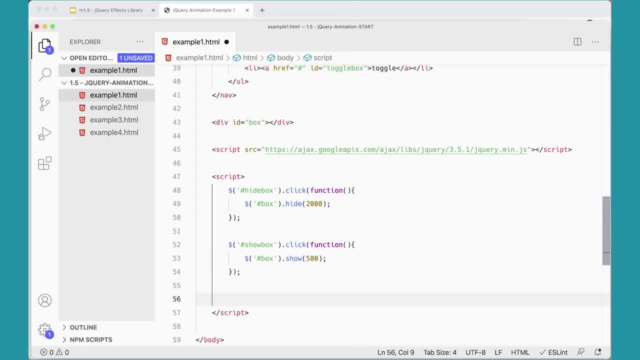 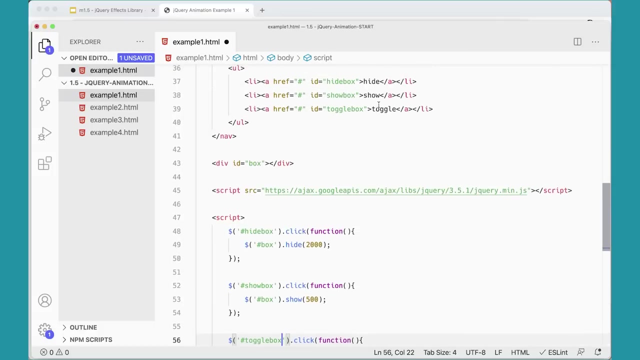 sake, i'm going to copy it, but i really recommend that you um, that you type it, so you get kind of used to that. so this is toggle box. it's this link here. it's this link up here, toggle box, and then down here we're going to do box and instead of show. 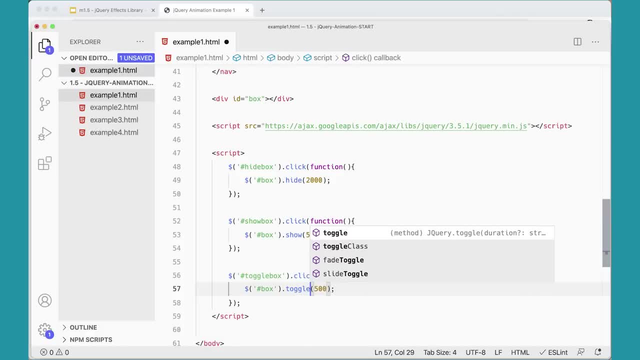 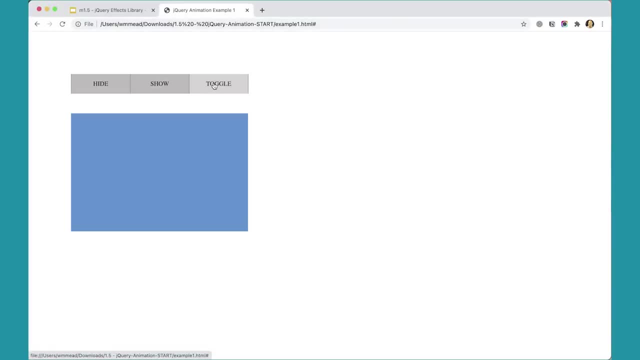 we're going to do toggle like that and you'll see over here, if i run this, it will hide it and it will show it. so this one does both remember. toggle is a helper function that allows us to do both hiding and showing, and we've seen that before. but now we can use. 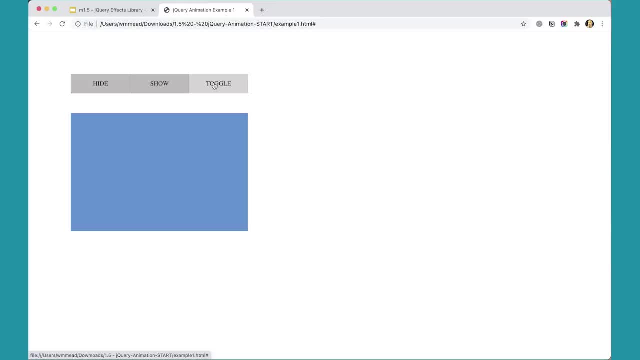 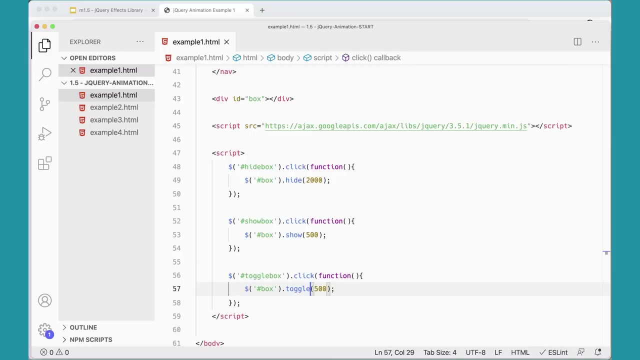 it with the effects library and do some animation with it. now, one of the really great things about these animations and doing this in in javascript and in jquery is that you have a thing called a callback function. so what you can do after the 500 here is: you can pass in. 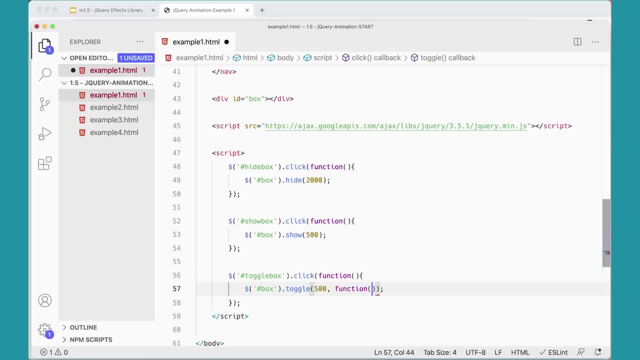 a function that runs with its parentheses and curly braces like so, and in here we could put alert, done something like that. so this function will run after this animation has been completed and in fact i'm going to make this a little bit longer so that you can really 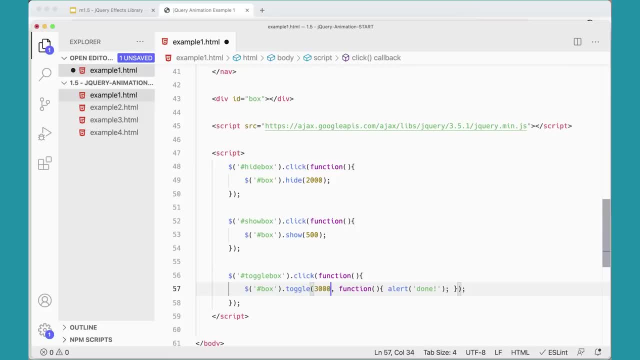 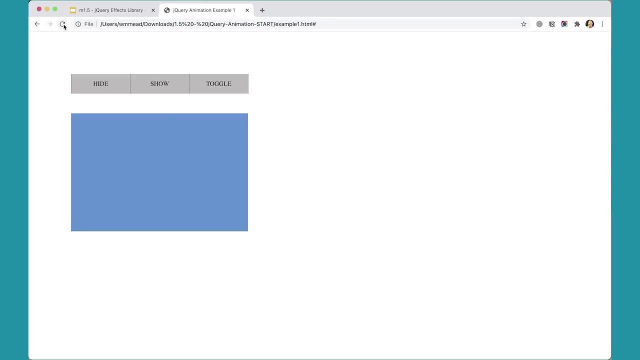 see that it waits and runs after the animation has been completed, and this is super useful, because sometimes you want to have a sequence of animations and when that animation is done, you want to do something else, something like that. so let's see how this works and the page does the alert. 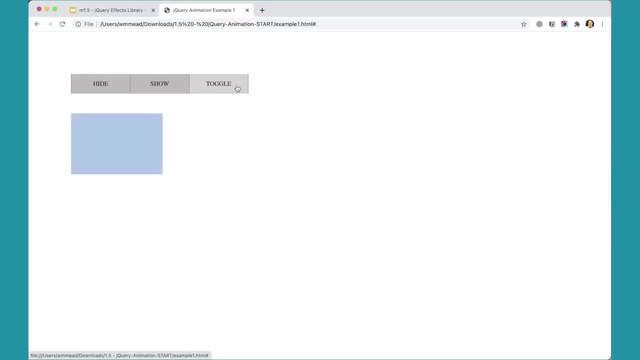 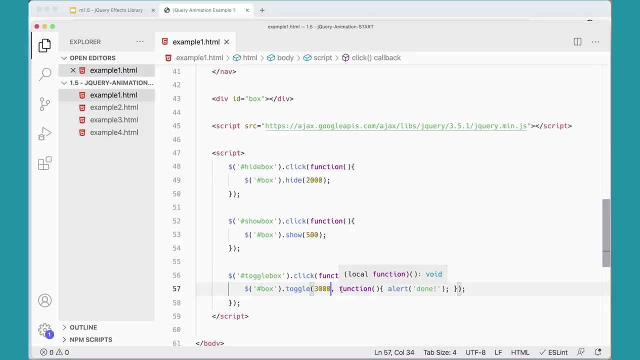 so that's really cool- and i could do the other way around as well- excellent. so with that, we are able to see that we can make these functions, these animations, and the animations can have a callback function that runs when the animation is complete, and this is super. 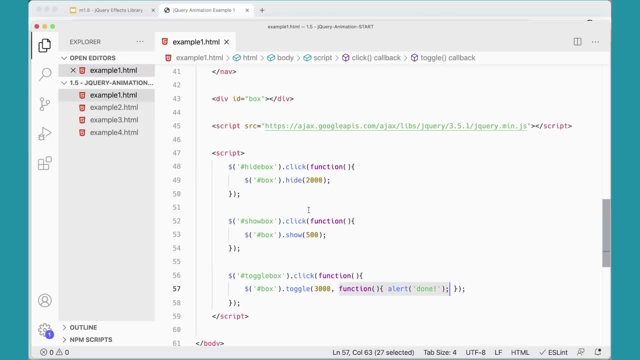 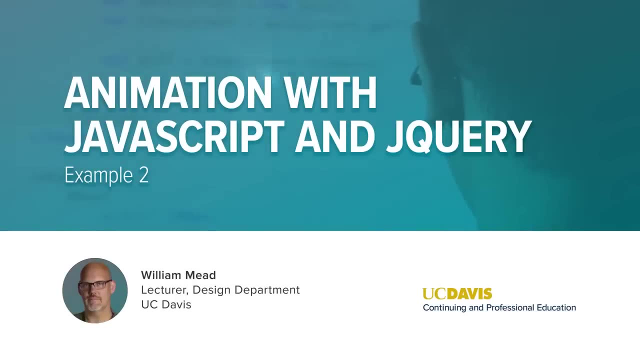 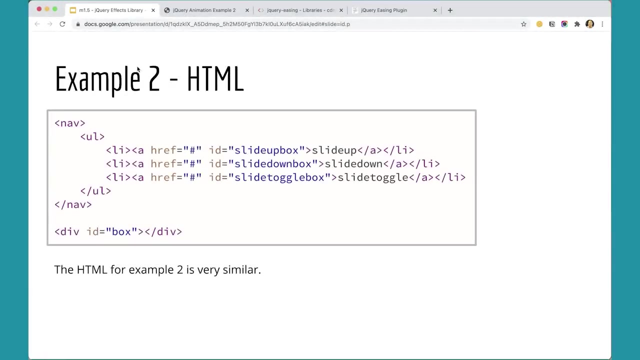 useful. let's take a little bit. take a look at the next example in the next video. let's take a look at example 2. open up the example 2 html file and you'll notice that it looks very similar to the first example. we have the same styling up at the top. 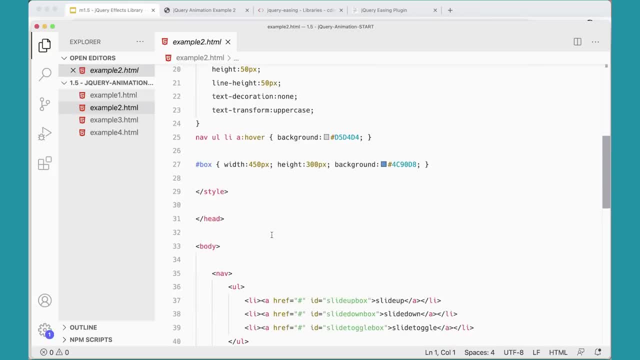 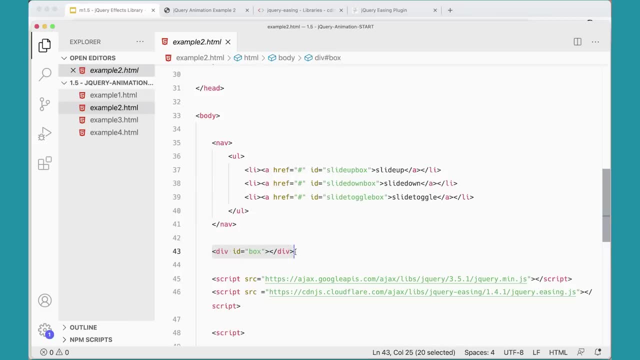 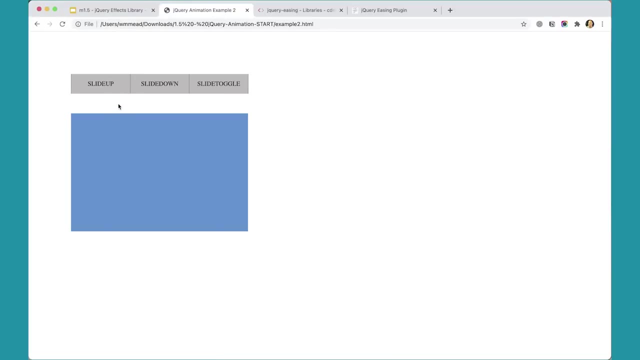 of the page. we have a box here, we have we have some navigation and then we have this div id set to box down here and it's just an empty div and you can see that it looks very similar here. but jQuery has some helper functions in for sliding up and sliding down. 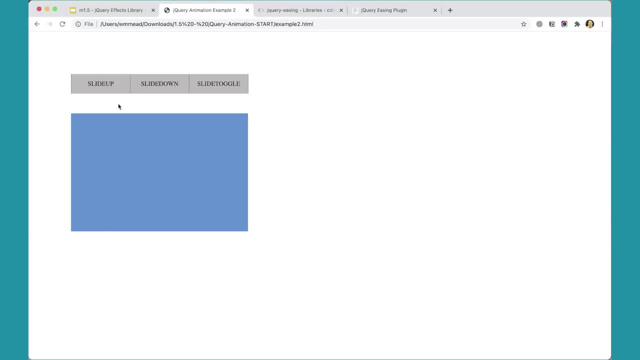 slide toggle because, again, these are common tasks, these are common things that we need to do in interfaces, so they created a method that does specifically this and that's kind of interesting and fun. so let's take a look at what we need in order to do this in our code. 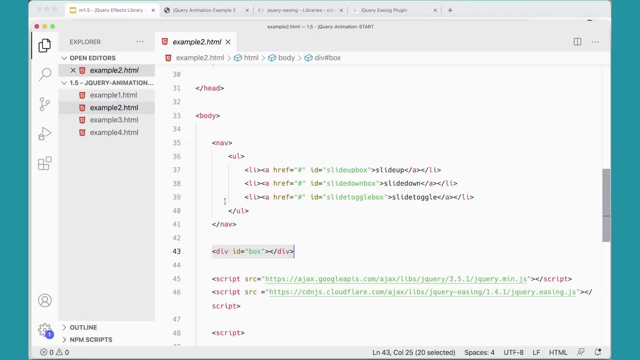 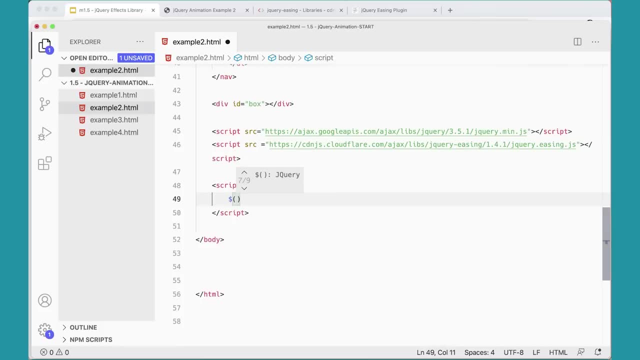 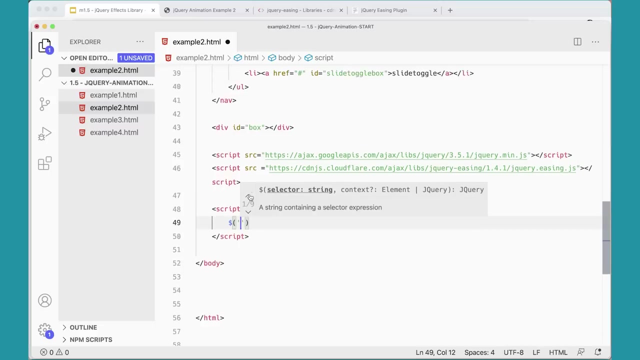 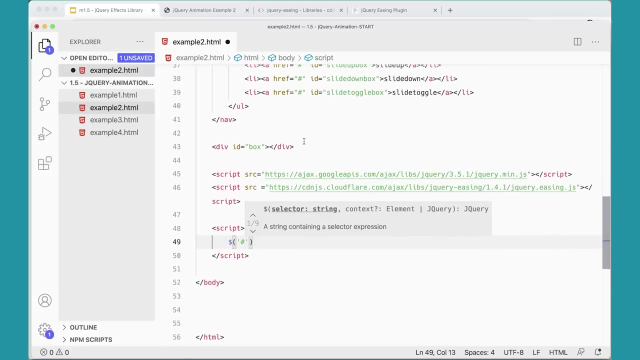 and the syntax is very similar to what we saw before. so what we're going to do is like we did before: we're going to use our jQuery object to go in and get our- our link here. so it's pound. I've got slide up box as a link here, so let's do that. 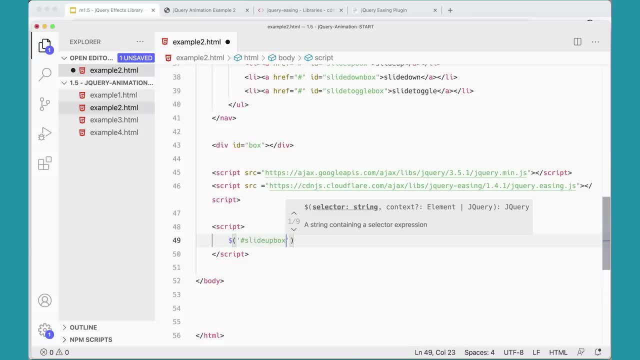 slide up box and we'll put a click handle there on that. so we're looking for dot, click, oops, like so, and then in here we're going to run a function with its own parentheses and curly braces, and then we're going to put our code. 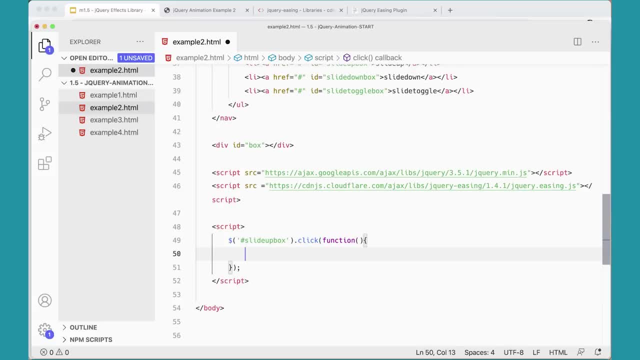 inside the curly braces there, just the same way we did before, and again as before, we're going to go get our jQuery object and get box, because that's what we're going to be moving up and down and then what we're going to use here for 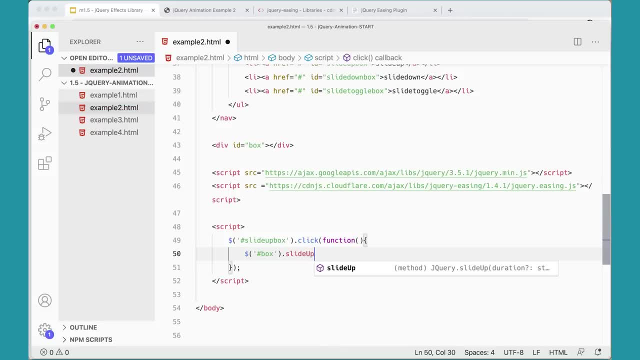 our jQuery function is slide up and again we can put in an amount of time or you could put inside quotes, you could put slow or something like that, and that will make that box slide up. so let's go over and give that a try. hopefully I did that right. 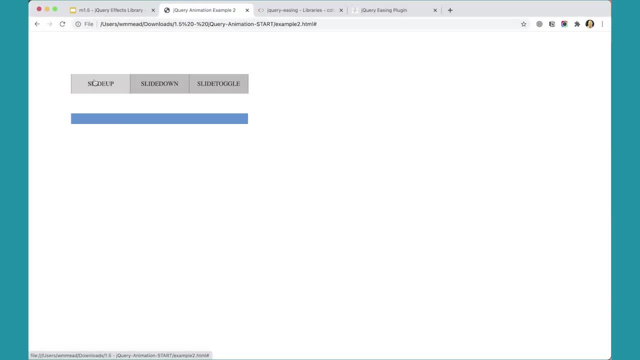 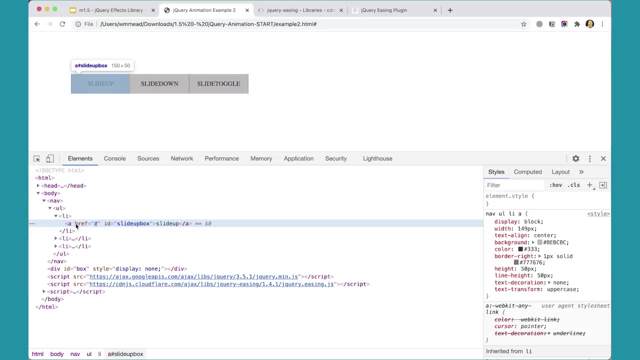 I think I did so. if I refresh this page and click slide up, it does that animation and it's interesting to inspect this and watch what happens here, um, actually on the actual box itself. watch what happens down here. slide up, you can see it very quickly went through. 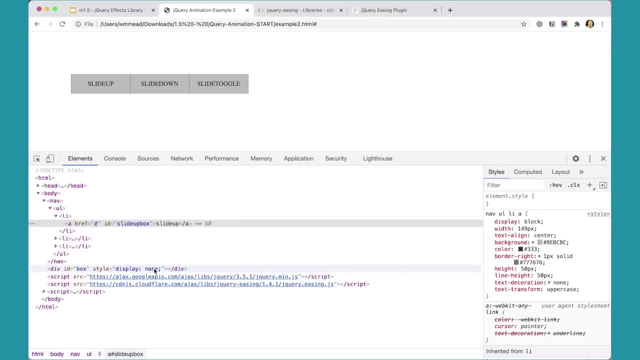 some settings in here, as it did that and ended up with display none, so that's kind of interesting as well. okay, great, so we can do that and we can do. the other ones look very similar, as you can imagine. so we've got slide up box, we've got slide down box and we've got 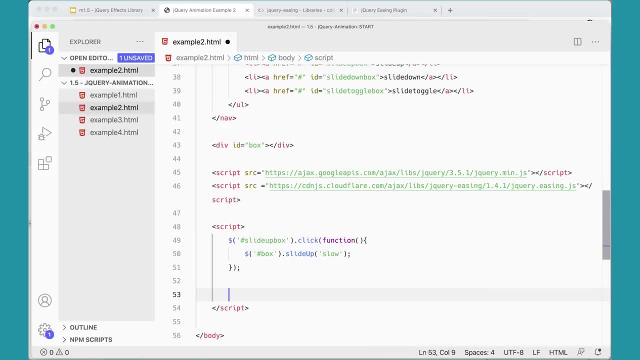 slide toggle, and they all work very similarly. so I can actually copy that, paste it, and I recommend you type it actually. but you know, for expedience sake, I'm going to just um copy and paste it and change this to slide down box and this is going to be slide down. 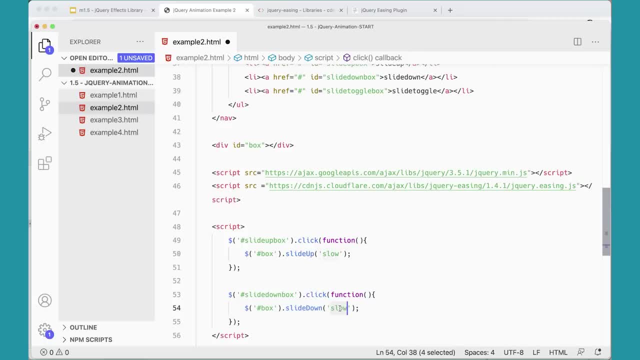 and I can choose an amount of time. we're going to do like two seconds, something like that, so we have kind of a longer time now. when you're working with animation, one thing to be aware of is that there's such a thing as easing an animation. 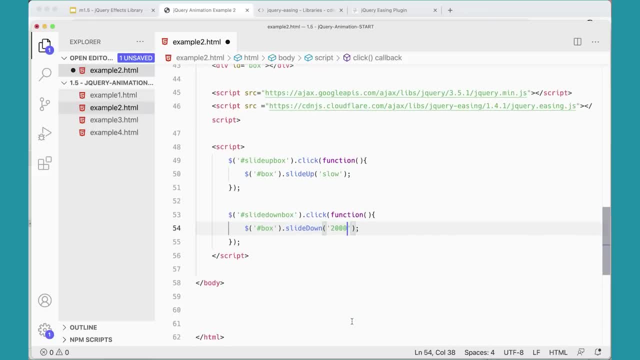 can run and it will run for the period of time. so this animation will run over two seconds, but it can run the exact same amount over those two seconds, which is linear easing, meaning that it's the same speed at the beginning as it is at the end. 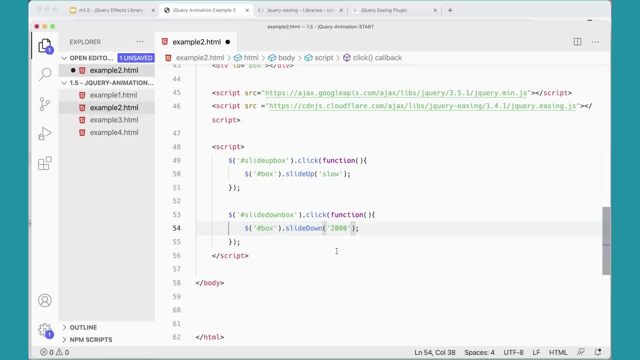 or you could change the easing such that it goes faster at the beginning and slower at the end, or slower at the beginning and then speeds up towards the end of the animation, or you can actually do easing in and out. where it starts slow, speeds up and then ends slow, or starts fast. 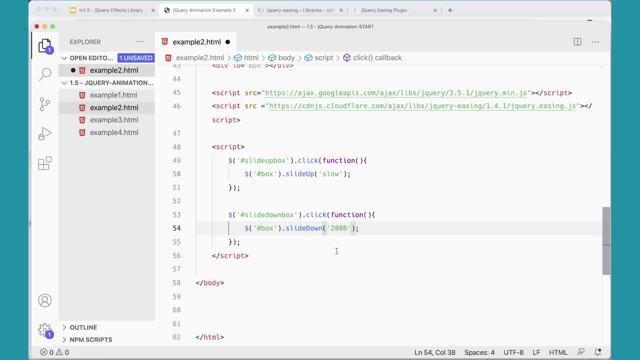 slows down and ends fast. you can do all of these different types of easings. jQuery has some basic easing built in and you can put in here in quotes, swing, and that will do a little bit of easing on this item and it's pretty subtle, so you don't really 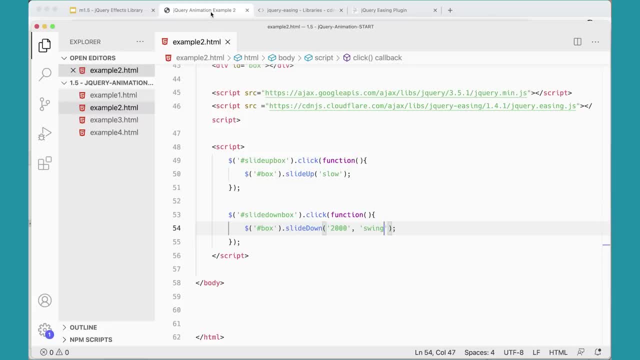 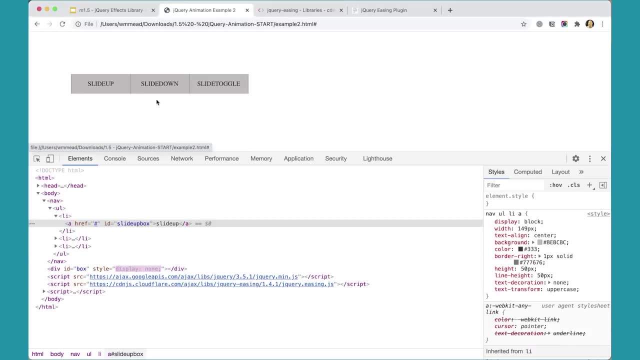 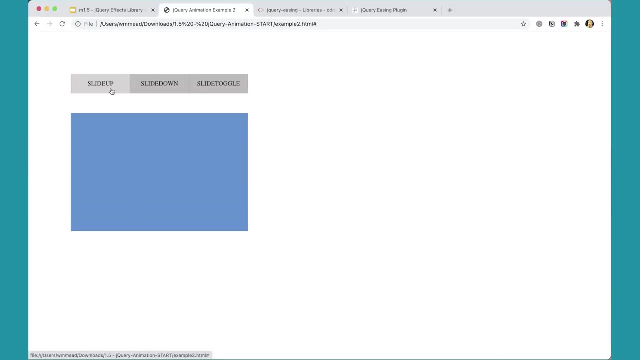 you might not really see it, but it will actually work. so let's go ahead and take a look at that. so slide up, slides up. I'm going to hide this. slide down does slide down, but it does a swing animation, so it's not the same speed. 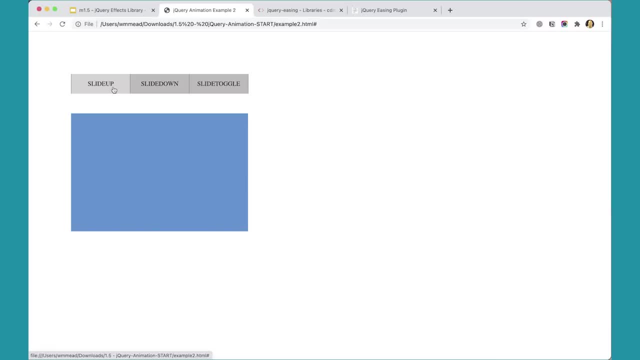 all the way through and you can kind of see the difference. it's hard to tell, but it is there. it's very subtle. now, jQuery has built into it just some basic easing, but there's a plugin and one of the strengths of jQuery is the plugin architecture. 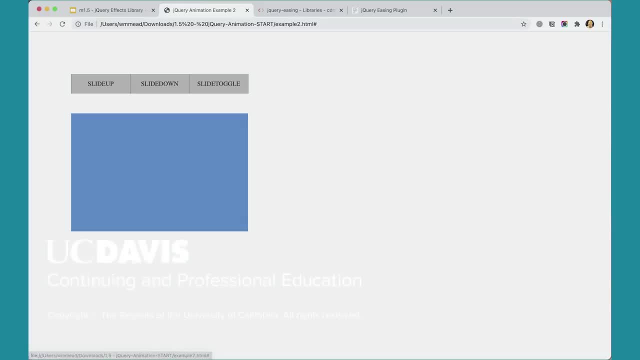 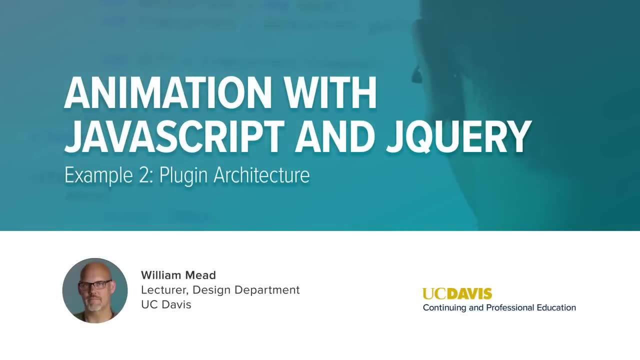 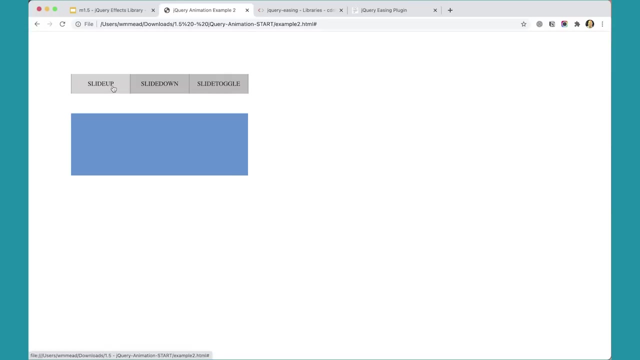 and we're going to talk about that in the next video. in the last video we added some easing to our function so that now it slides up sort of just using the linear easing, but slide down is using the swing easing, and easing can give your animations a little. 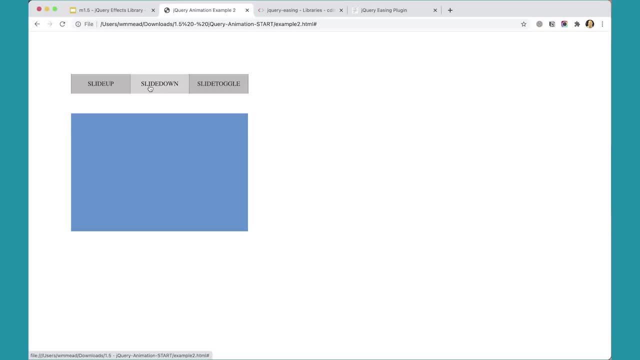 bit of personality. they can make them seem a little bit less mechanical when the speed of the animation is not always the same all the way through the animation. but the easing that are built into jQuery don't really give you a lot of options. they're very basic, so 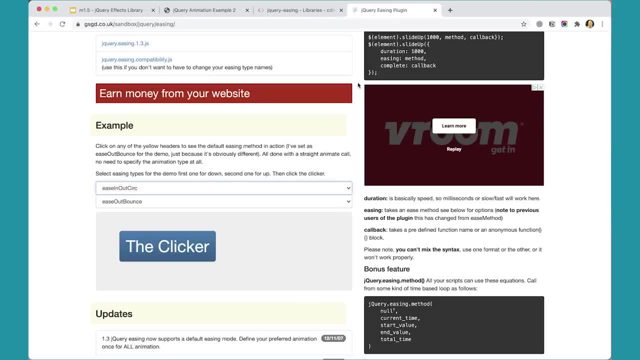 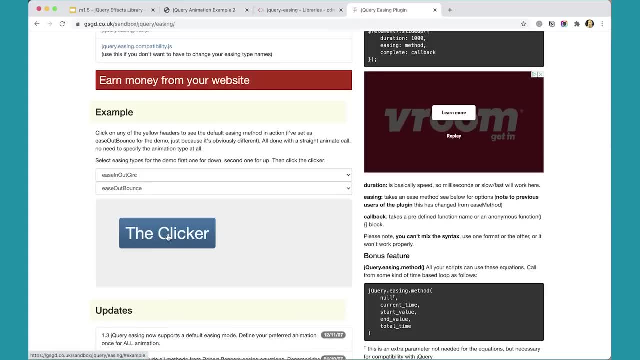 there's an easing plugin over here that we can use and it allows you to choose different types of easings so that you can actually do some different types of things with this, and you can go through and try some of these different settings here to see what they actually do. 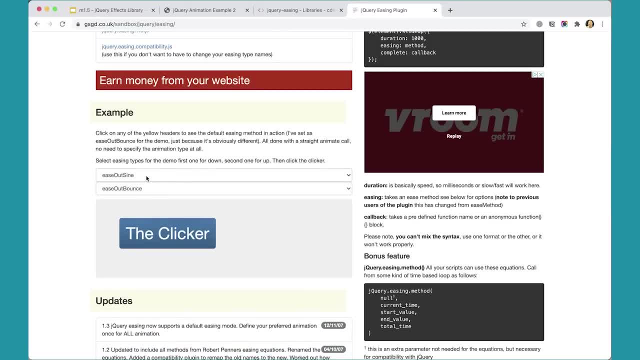 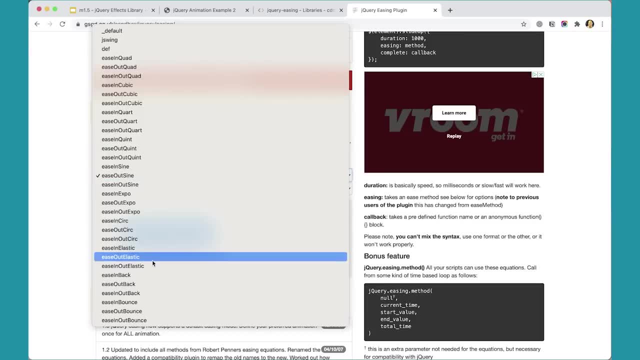 so ease out will affect the animation at the end, where ease in will affect the animation at the beginning. ease out and in will affect the animation at both ends. so we've got ease in and out, um, ease in out, you know, we've got a whole bunch of them in here. 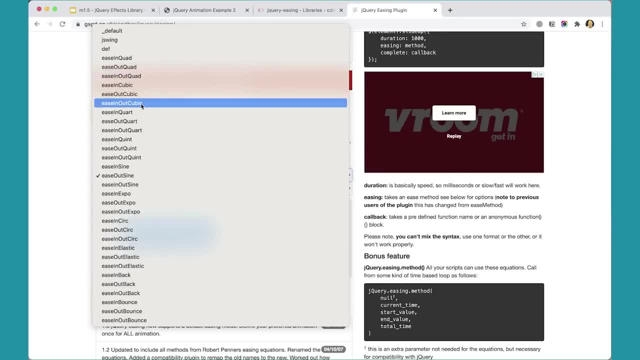 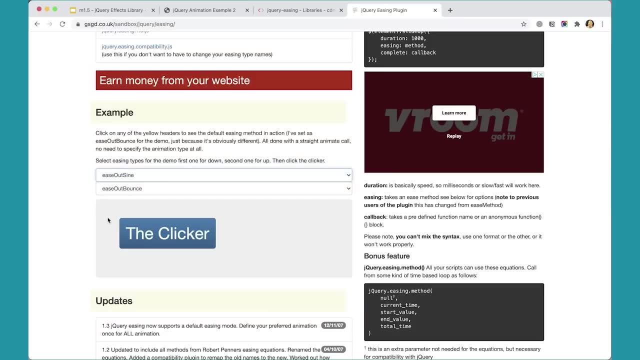 for all of these different in ease out. we can use in ease out ease in all these different animations in here, but in order to use this, we have to plug in this plugin and jQuery has a plugin architecture that allows you to add more functionality to javascript. to. 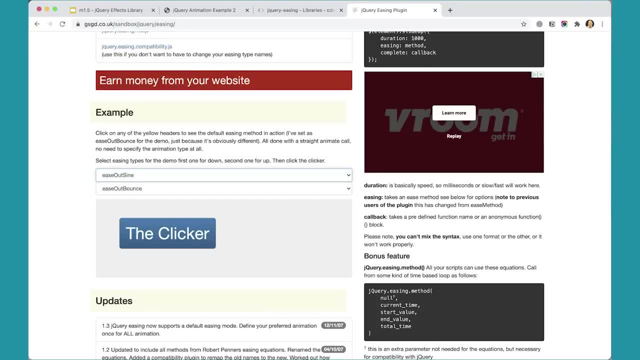 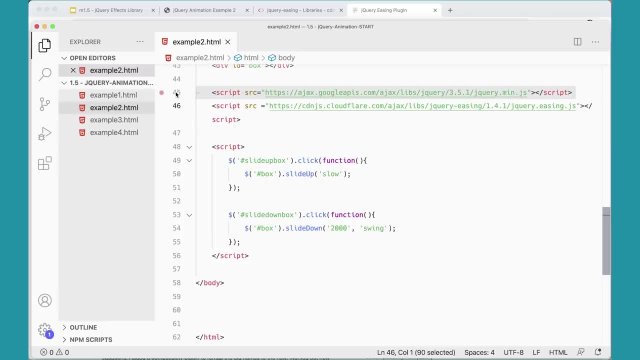 jQuery, and you can see over here on our file that I've already added the plugin. so the way this works is: first we need the jQuery library, then you need the plugin and then we use it in our script. so down here I'm going to do the third. 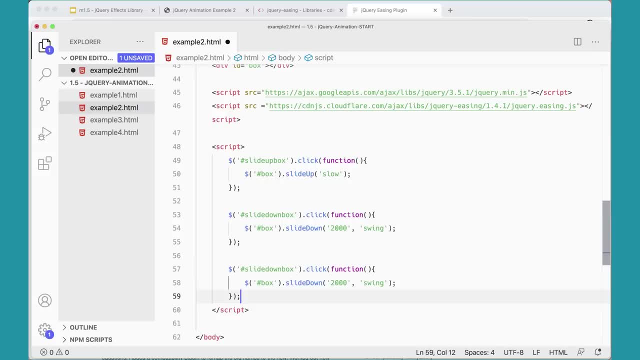 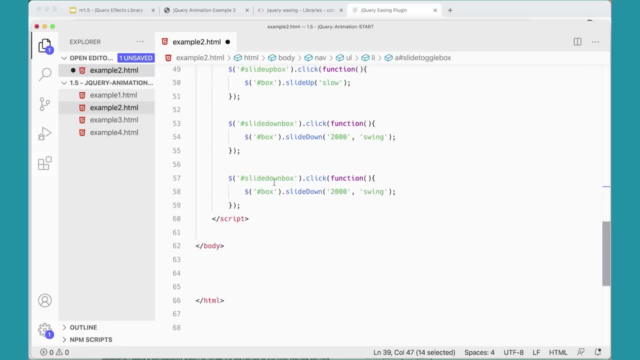 animation here for slide toggle, which we're going to use, this ID. so we'll grab that ID and down here, instead of slide down, we're going to do slide toggle, which will open it and close it, and here we can use some of the other easings that we. 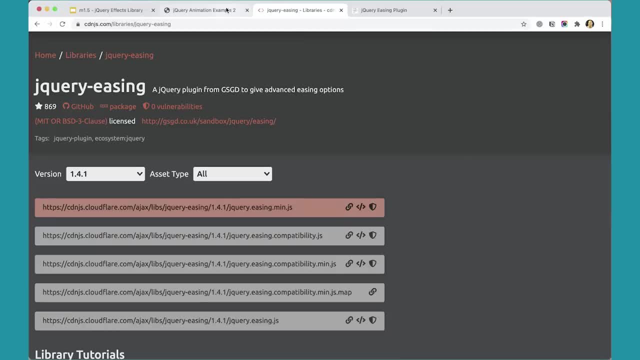 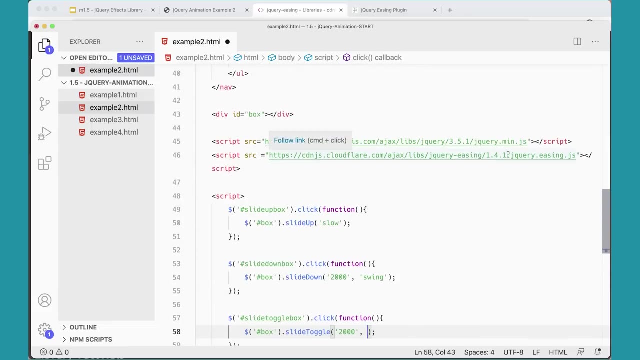 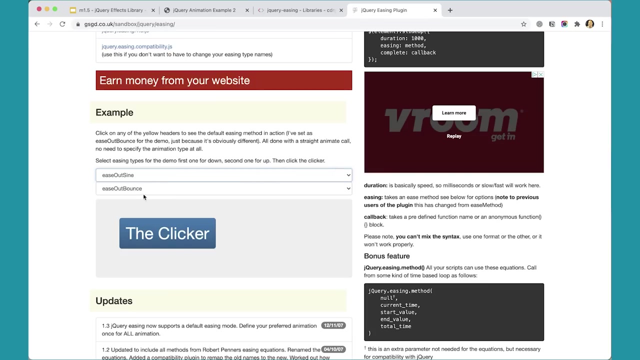 find on this website here. this is where I got the, the, the easing plugin on the CDN that I put into here. so that's where that came from. so that comes from this website here. but we can use the easings that we see here. so if I want an ease out bounce. 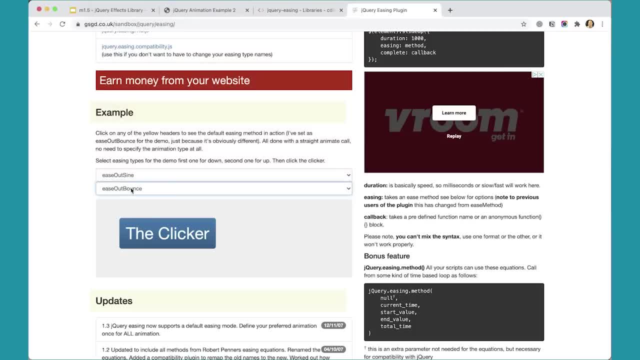 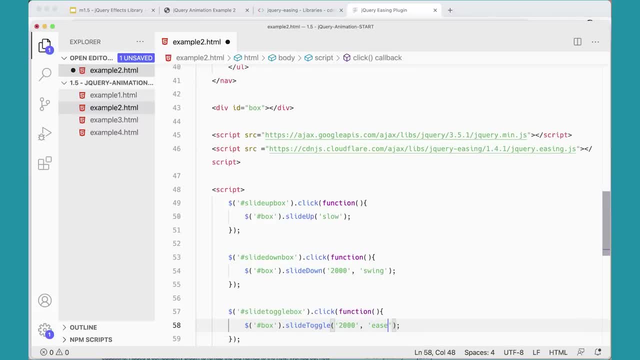 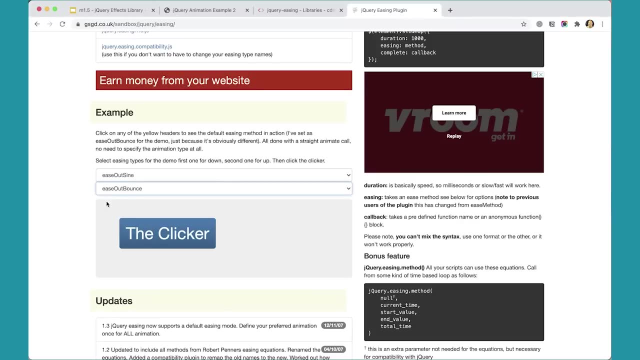 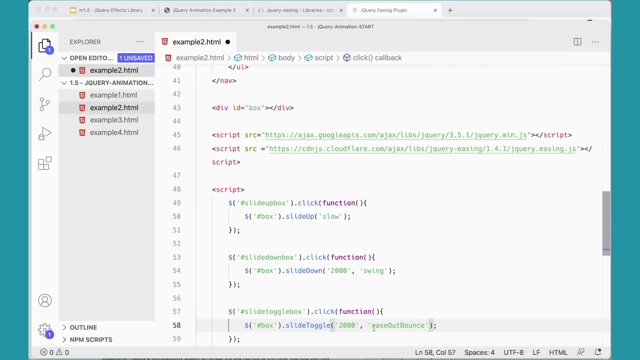 I can actually use that animation if I want over here. so let's give that a try. ease out, bounce and make sure you spell it right, the capital letters and everything. ease out bounce, so make sure you spell it all correct and that you get the correct capital letters. make sure you put it inside. 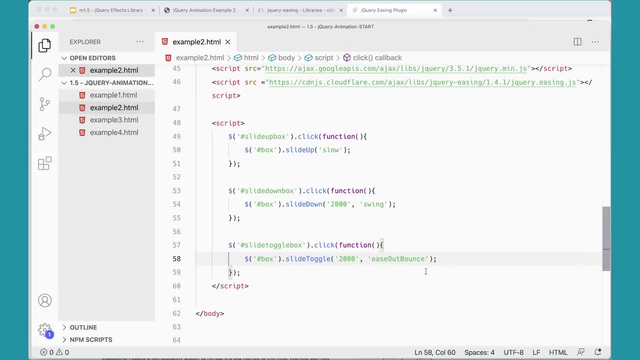 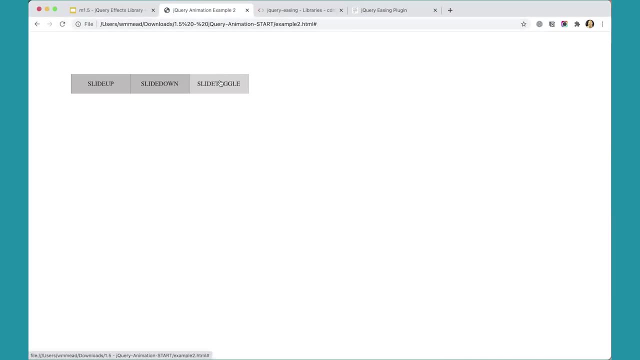 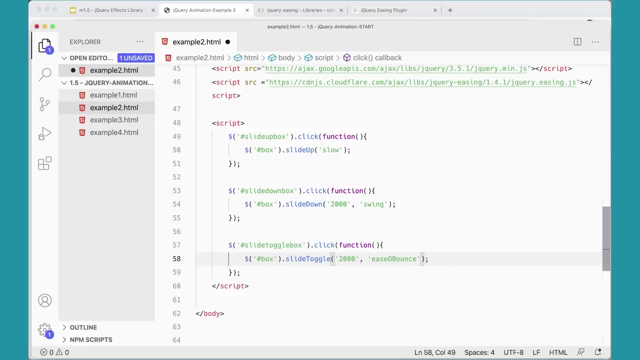 the quotes and so on and so forth. so if I save that and then come back and look at my example here and click slide toggle, you can see that it does this bounce, which is pretty interesting, and or you could do ease in bounce to get the bounce on the opposite. 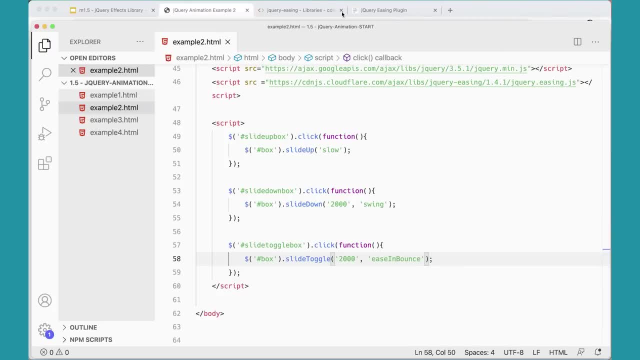 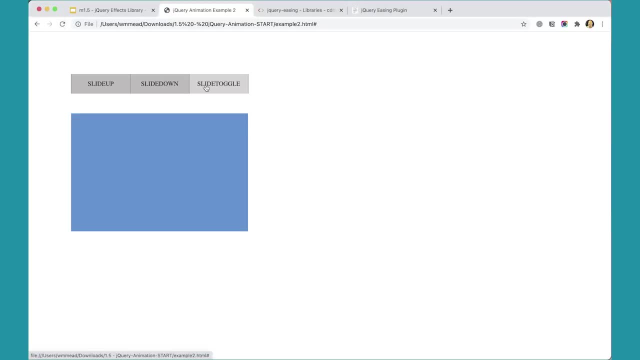 end of the animation, which might look a little weird, but let's give it a try. so it's doing the bounce first and then it's finishing the animation, which looks a little weird, but you get the idea. and you could try some of these other easings and see. 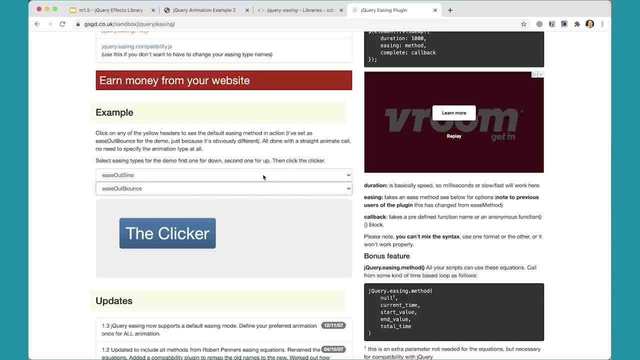 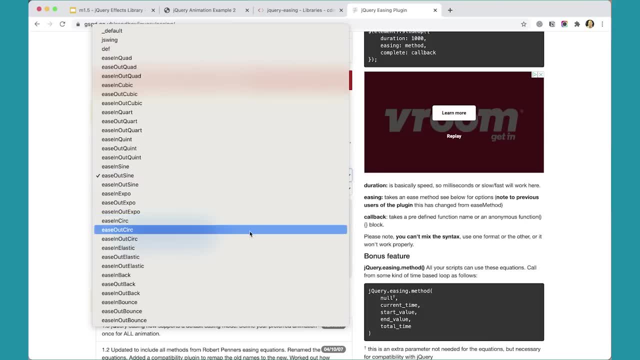 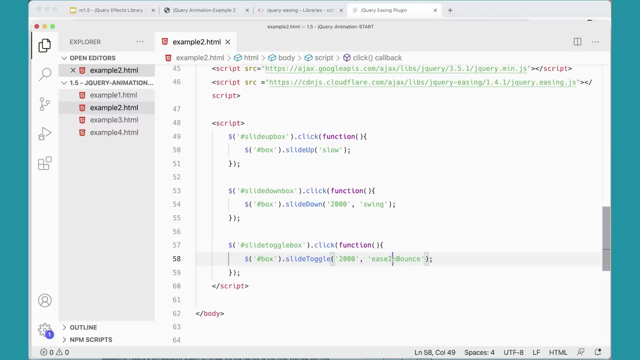 what sort of personality you can get. so I really like the ease out circ ones. where'd they go? yeah, ease in and ease out circ. you can give those a try. so let's see what we can do with that over here. ease in circ and again at two seconds, that's. 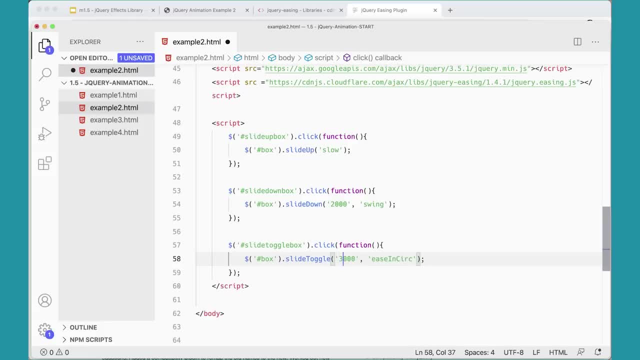 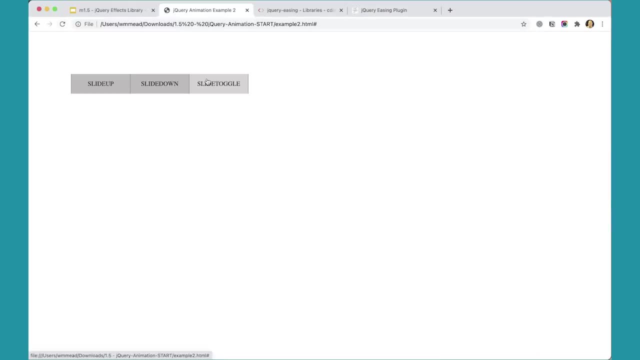 pretty slow. you can even slow it down more if you wanted to, to really sort of see it, and set that to three seconds, you can see how it changes the animation by either slowing it down or speeding it up. I think this one's speeding it up as it gets. 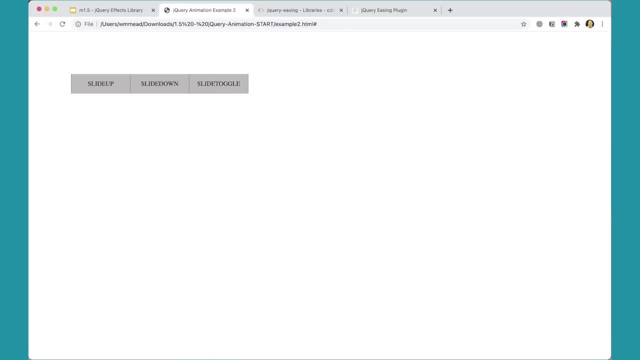 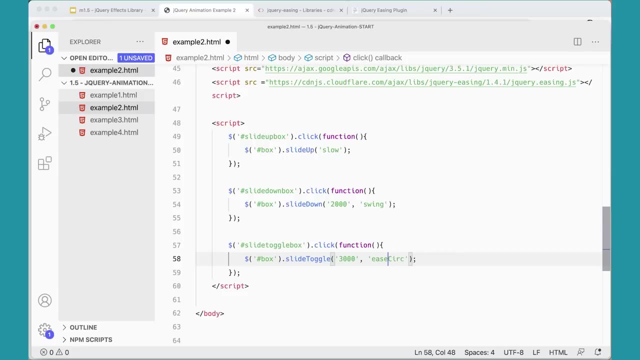 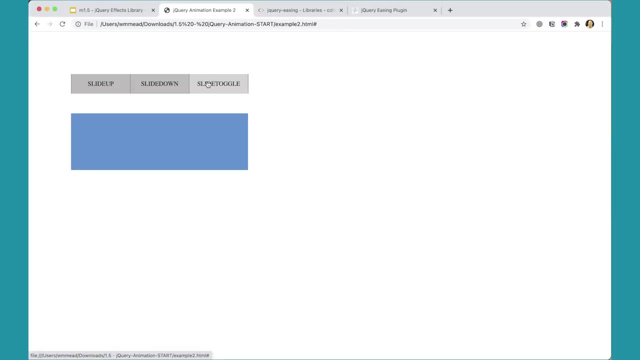 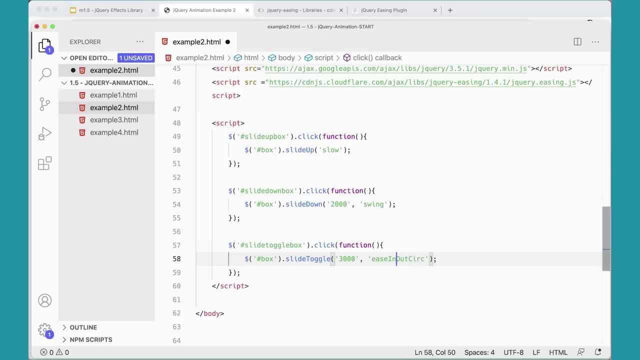 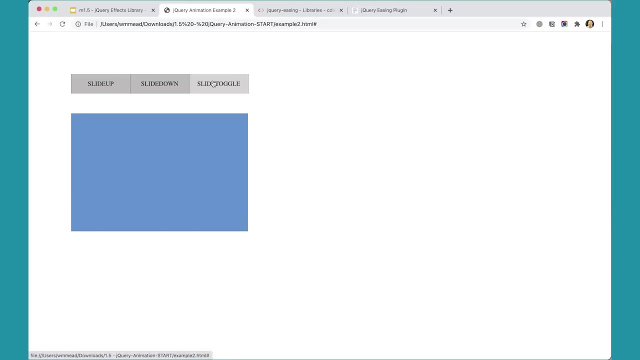 to the end of the animation, let's come back and try ease out circ. so that's starting fast and ending slow. it gives the animation a little bit of personality, as it does its thing. that's pretty cool and you could try ease in out circ and it's hard to see. but 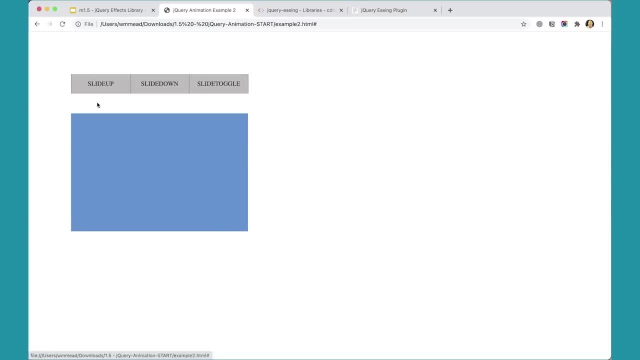 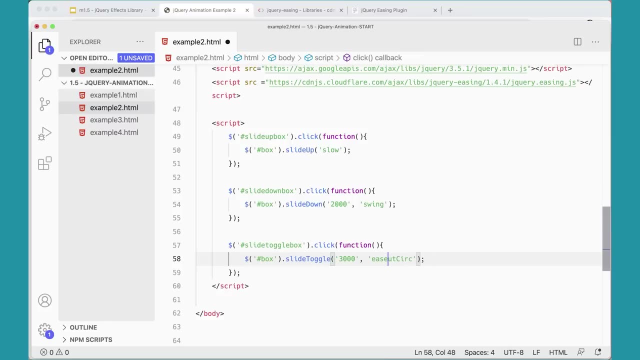 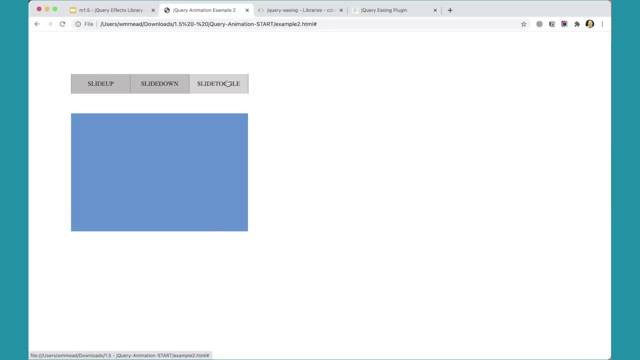 it is doing something there. so try these different animations, you'll notice if you spelled them wrong. if I do ease out circ like that, then it won't work quite right at all. if you inspect, you'll see that I'm getting a whole bunch of errors there. 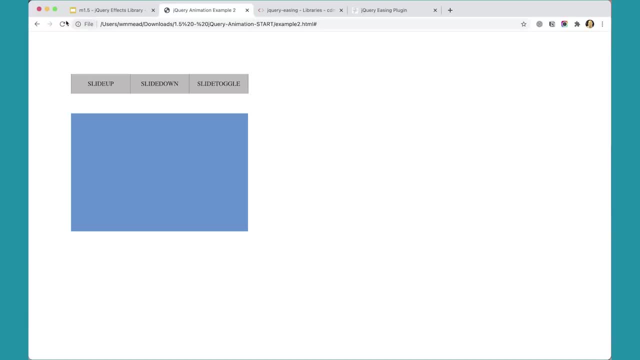 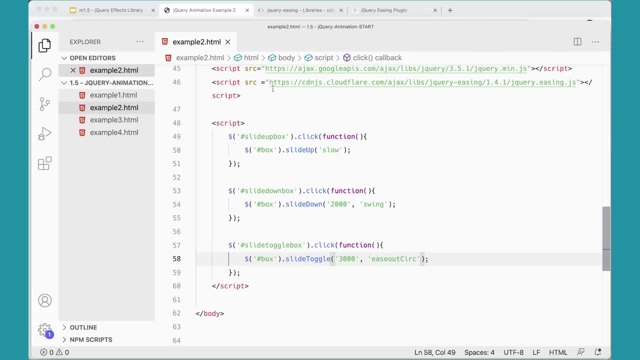 because I've spelled that wrong, so that's not helpful. also, if you were to forget this easing library, you'll notice it won't work if I just comment this out for a minute and try ease out circ, even if I spell it wrong. oops, you'll notice it won't work, right. 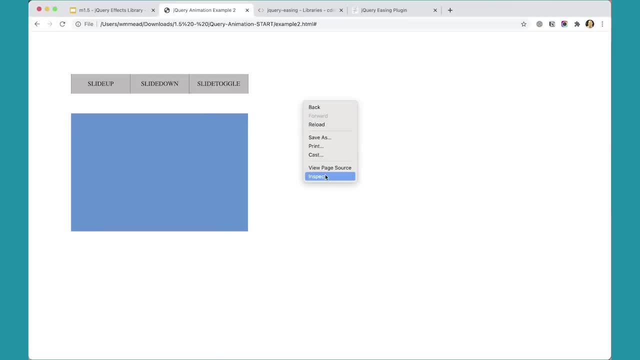 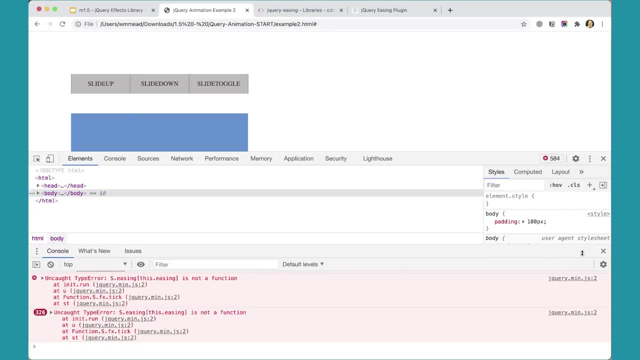 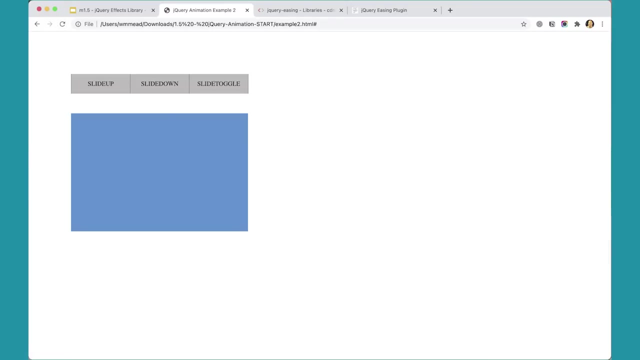 or work at all really, and if I do inspect, you'll see that I have a bunch of errors cooking here because it doesn't know what to do about that, because it's not a function. so in order for this easing to work, you have to really make sure that you have the easing plugged in. 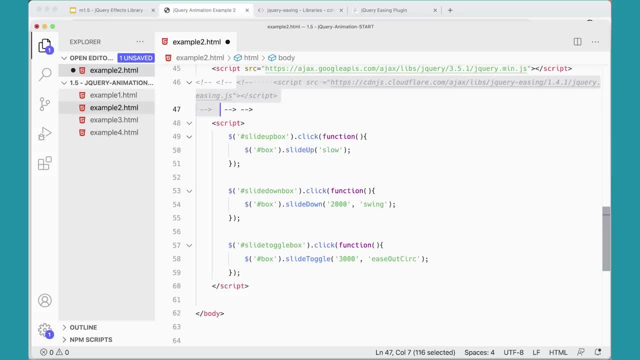 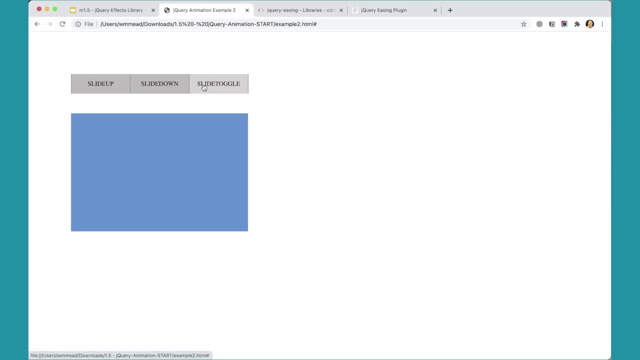 plug in, plugged in and that. there we go and that you're spelling these correctly. ease out, circ. let's give that a try again and you can see that it's working nicely. okay, great, so that will all work and that's awesome. one last quick thing here. 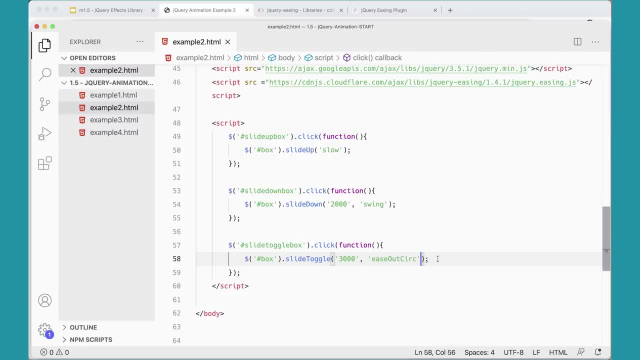 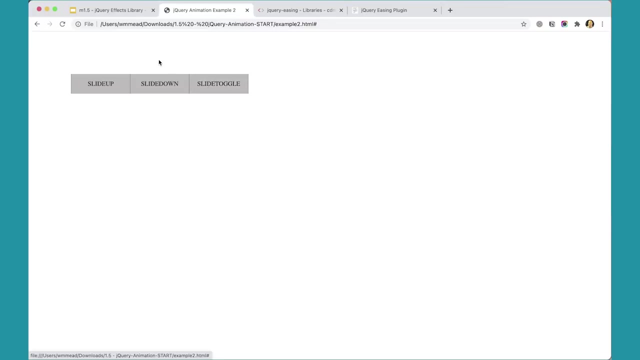 before we're done with this video is: you can also add the callback function after the easing. so I could add a function here and say done, and you'll see that when that easing is finished, when that animation is finished, that callback function will fire. oops, sorry. 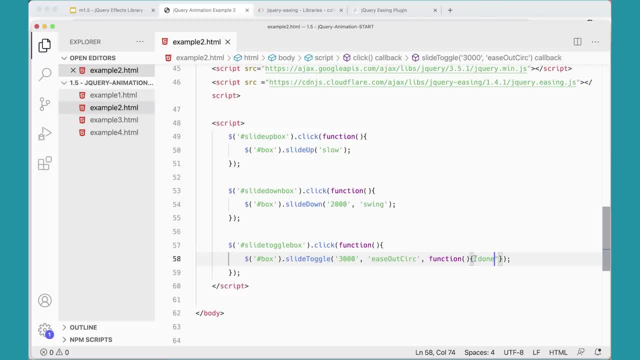 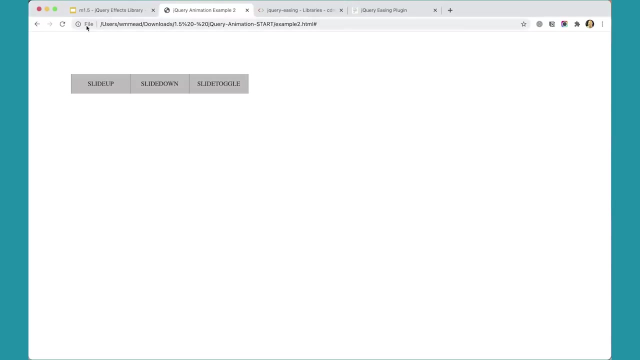 I think I did, I just did done, but I need to do, I need to do that right alert done like that, now it'll work and it comes back and it says it's done, so that's working, great, okay. so that gives us a lot of information. 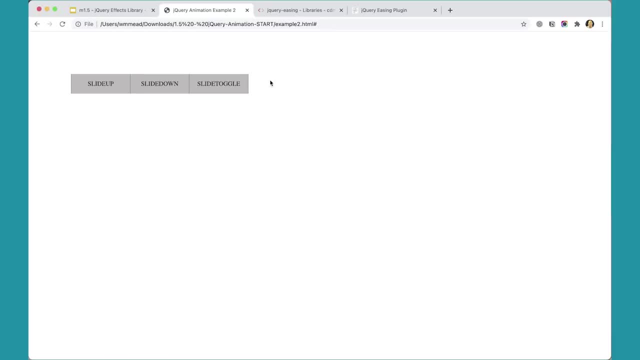 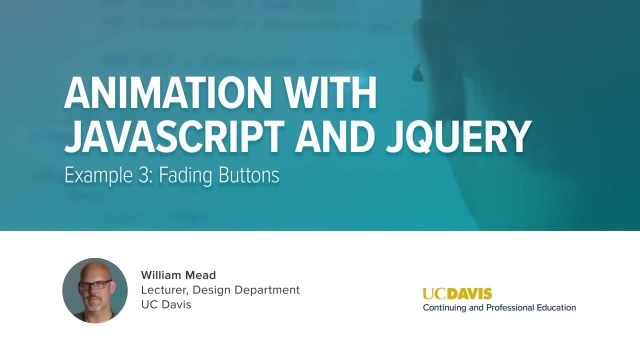 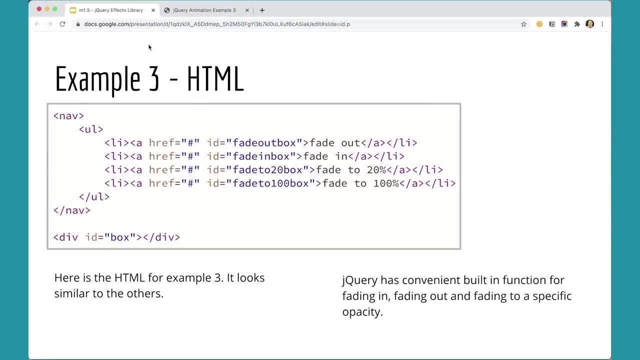 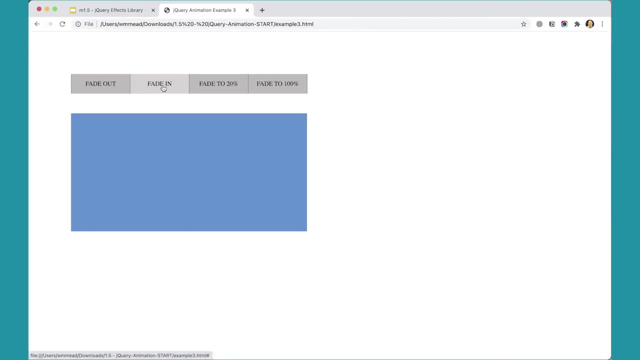 about how to work with these built in animations, and we're going to do more in the next video. in example 3, we'll look at something that's similar to the other two, but just slightly different. it's got four buttons and we can use some built in functions. 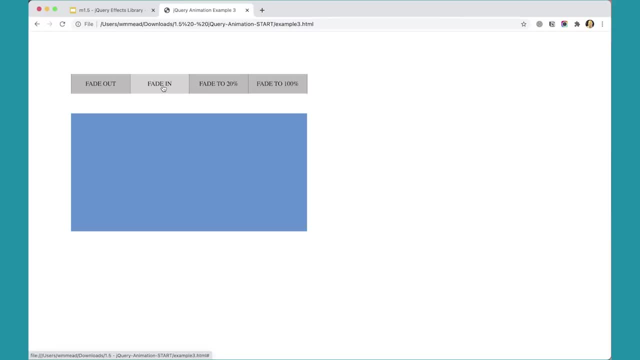 in jQuery to fade objects in and out or to fade them to a particular percentage of opacity. so here I have fade out, which will fade it out completely. fade in will fade it all the way to being visible. but then I have fade to 20%, which will fade it. 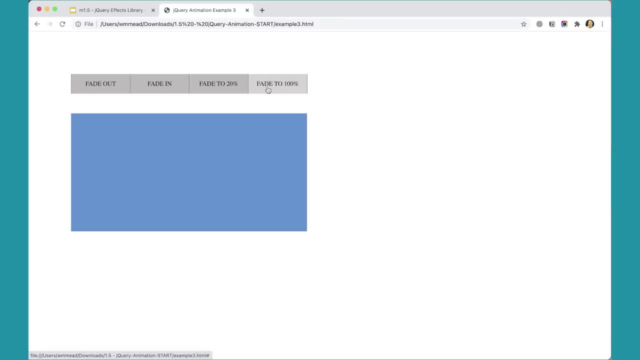 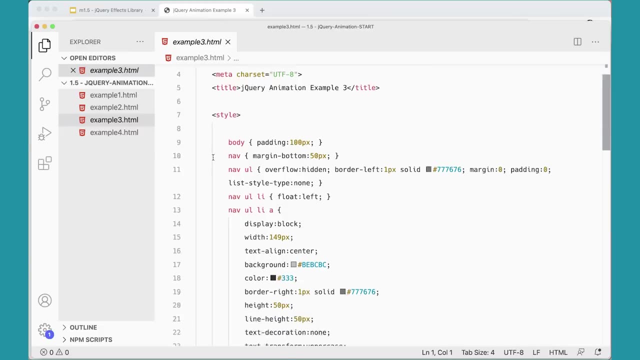 to 20% opacity and then fade to 100%, which will fade it all the way in. so let's take a look at how we can do that over here. I have example 3 open and you can see that I have much the same styling up at the top. 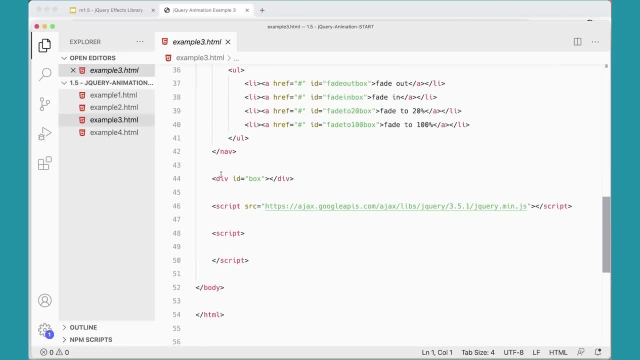 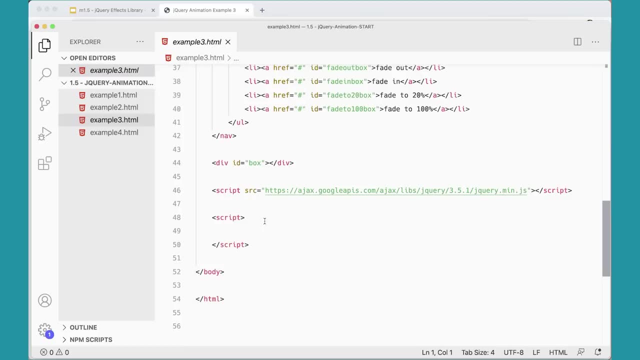 of the page, as well as my navigation here, and my jQuery library is plugged in. I don't have the easing plug in here, but you could add it if you wanted to add some easing to these as well. so here we're going to just go ahead and 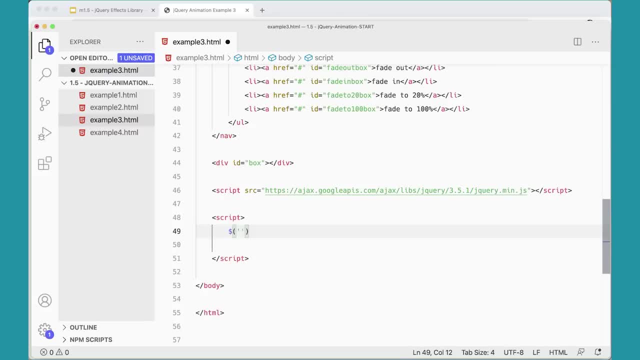 do what we did before with getting our link pound fade out box, which is this first link up here, and we're going to add our click handler to it: click and then we're going to pass in our anonymous function that runs when you click that thing and in here we're going to go get. 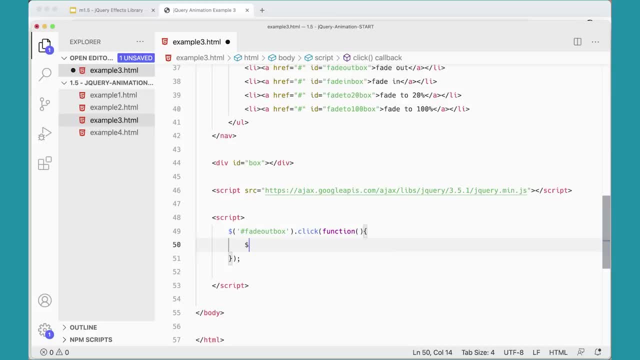 our box. so again, we use our jQuery object to get box oops, pound box. sometimes students make mistakes here and they forget to type the pound. so if you do that, make sure. if it's not working, make sure you have pound box in here, because that's a common mistake. 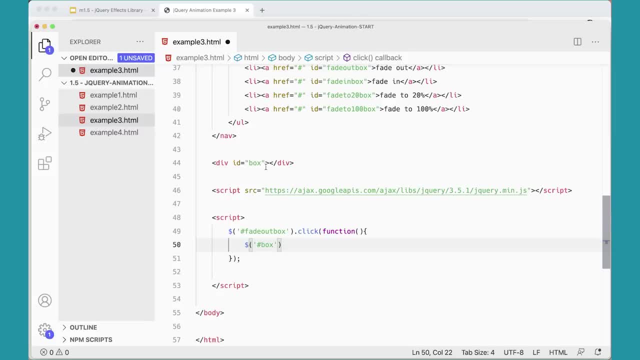 that I've seen. so it's pound box to go get this div ID box here and then we're going to do- I believe the function is fade out, because we're fading out the first one and again we could put in normal or you could put fast. 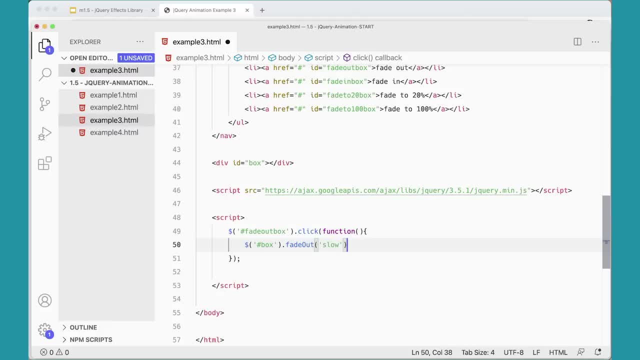 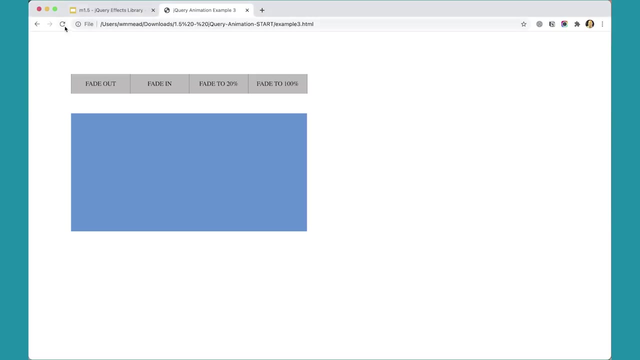 or you could put slow, or you could put a specific number of milliseconds: 3000. 3 seconds is kind of a long time, but we could actually give that a try. so you'll see that will actually work over here. we can fade the box out, fade out. 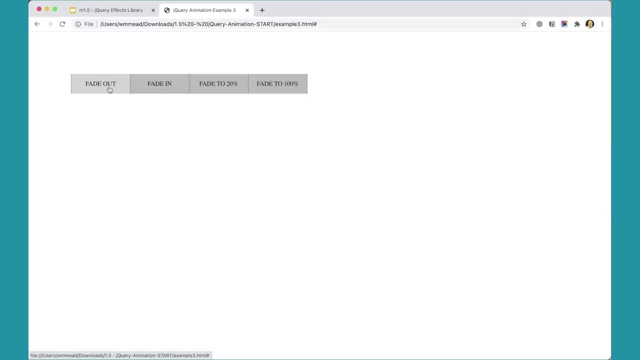 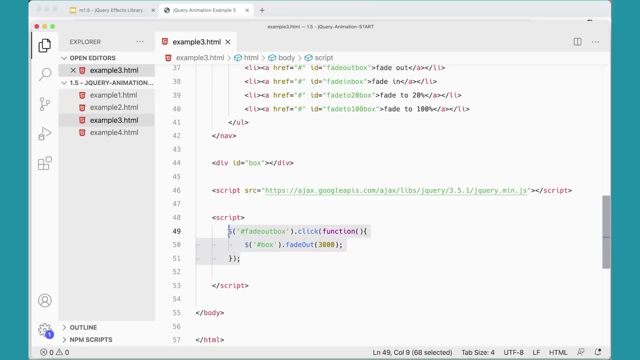 in over 3 seconds it will become invisible. so that works and that's great. and we could do fade in as well, so I can copy that and paste it or just type it again. it's always a good idea to do that, but we're going to use this. 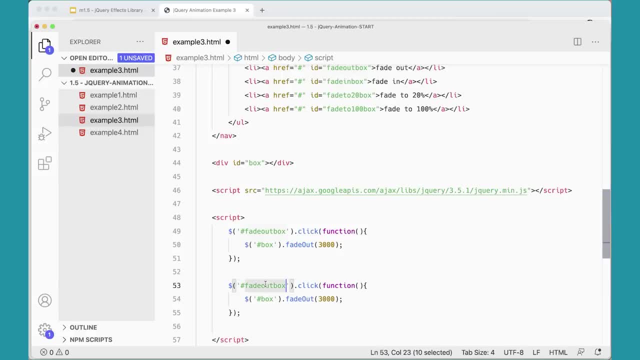 um ID. instead, and instead of fade out, we're going to fade in and I could do 3 seconds and you could do the easing swing. it's going to go in quotes swing and then you could also add a callback function, function and that's parentheses and inside. 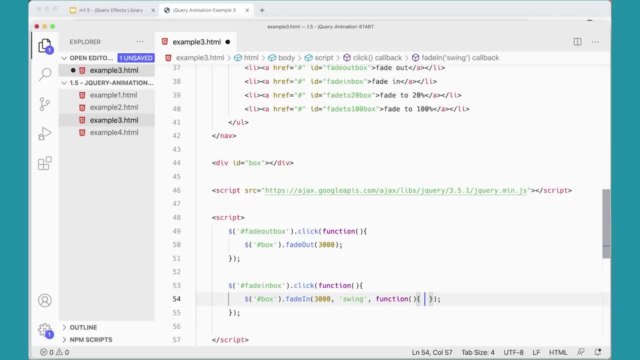 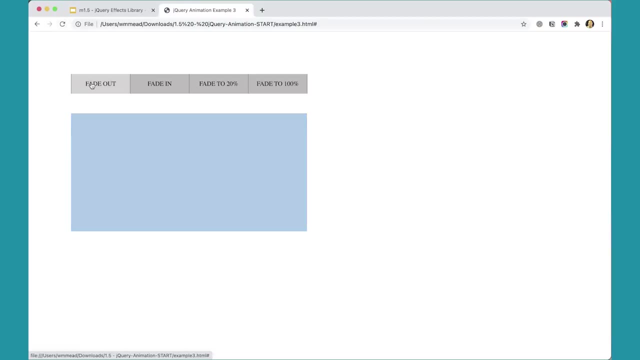 the parentheses we can add: I mean inside the curly braces, we can add an alert that says done. and so now we can fade the box out and we can fade the box in. let's give that a try. fade out and it fades out over 3 seconds. 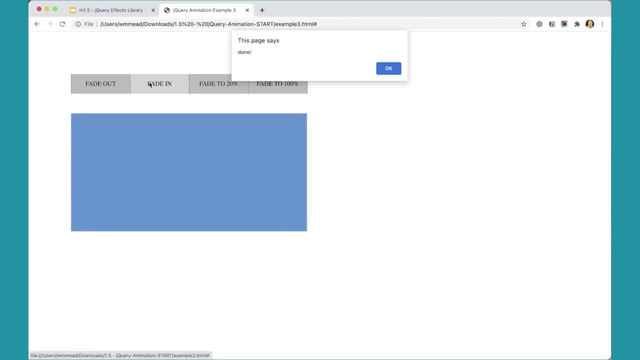 fade in. it will fade in over 3 seconds, and when the animation is complete, it runs the alert and says that it's done. so that's great. we can do all of that, okay, cool. so now we just need to add these last two here and we can look at. 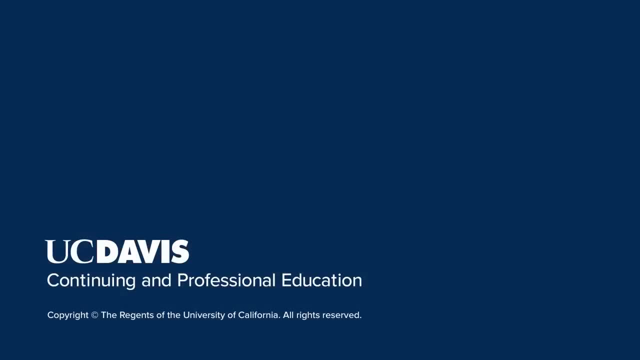 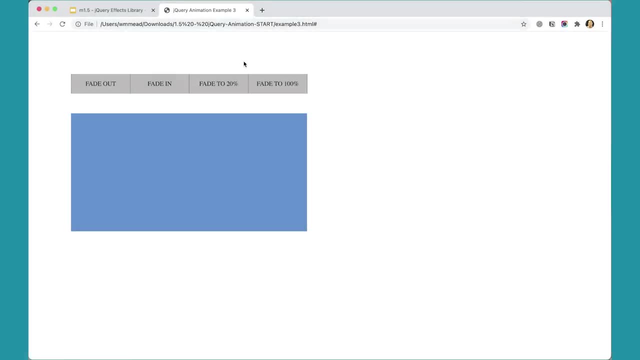 that in the next video. in this video we'll make these last two buttons work, and with that there's a fade to method that we can use in jQuery, so let's go see how that works. so here, just as we've done before, we can add a new. 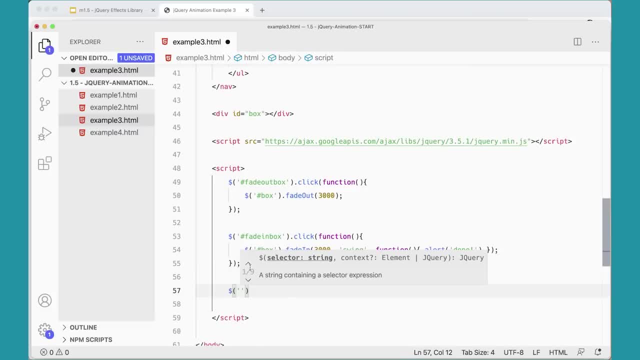 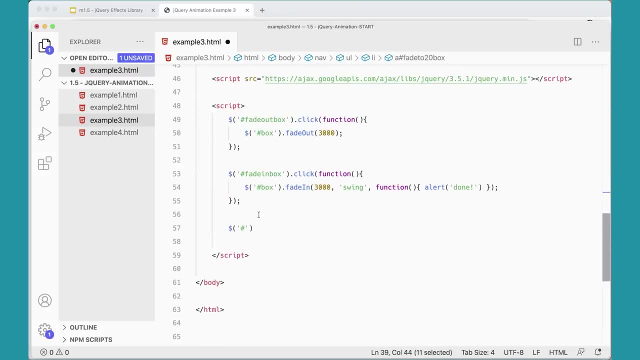 event handler for when you click the the button that has fade to 20 box on here. so I'm going to paste that in just to make sure I spell it right and we'll add a click handler. and again, I recommend typing this just to get used to the syntax. 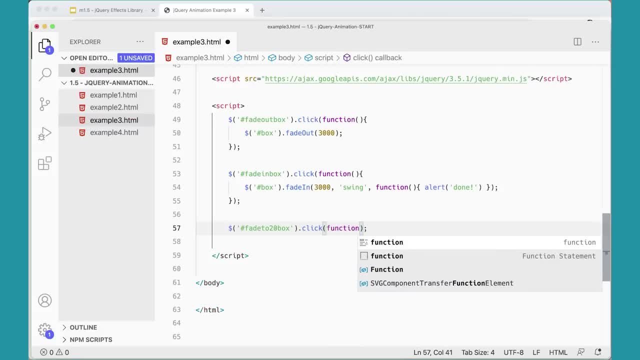 and then in here we'll add a function that runs when you click it. it's just an anonymous function, and what we're going to do here is, once again, we'll go get pound box- don't forget the pound sign- and we're going to use the fade. 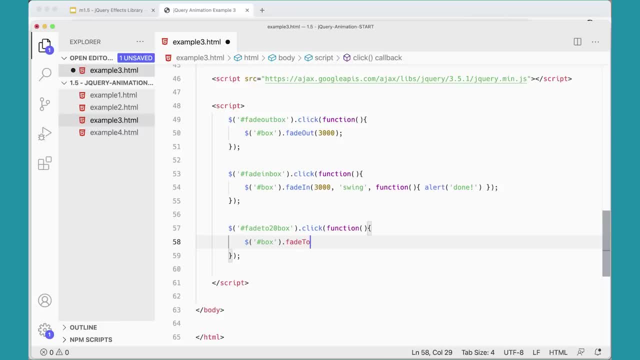 to method. see it even comes up here: fade to and we're going to fade to. the way this works is we're going to put in the amount of time. so we'll do again. I'll do 3000. it's kind of slow but gives us a sense of what that. 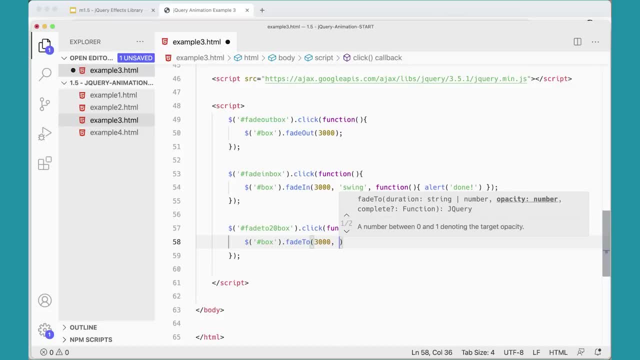 is. but then the second number it takes is a duration, an amount. it takes the duration. that's the first number. the second number is how much it's going to fade to. we want to do 0.2 like that, and now that should actually work. so let's go over and check. 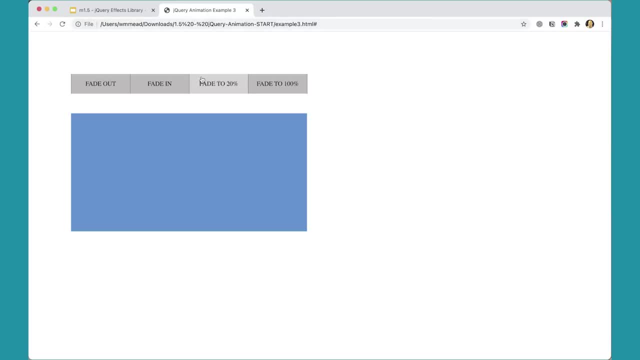 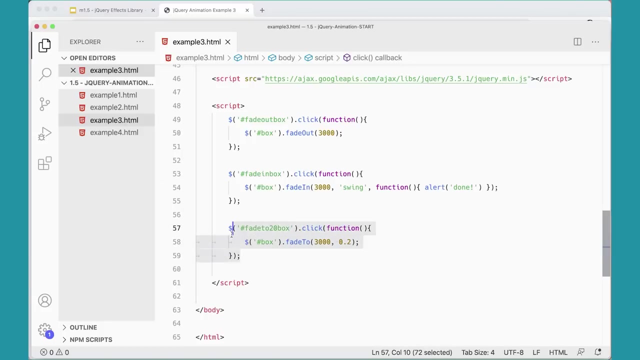 it out, probably refresh this and click fade to. it fades down, but it doesn't fade all the way down. it fades to 20%. so that's really pretty cool. so we can do that and then we can do the fade to again for the last one. 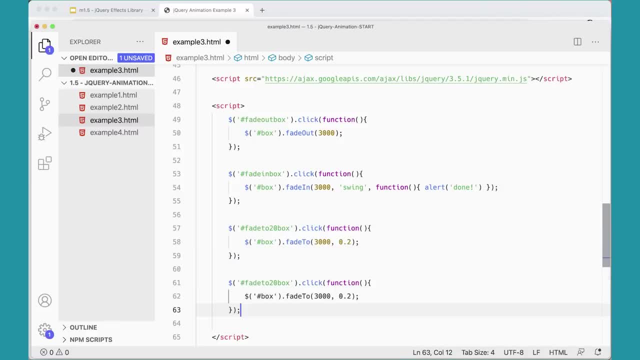 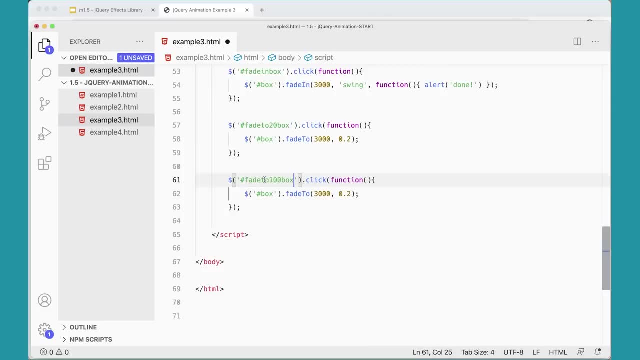 so I'm just going to copy this and paste it and we're going to use this link fade to 100. so when you click the fade to 100, it's going to fade to 1. so the opacity is a number between 0 and 1. 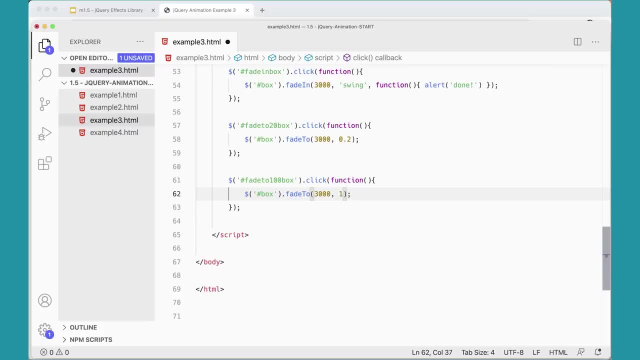 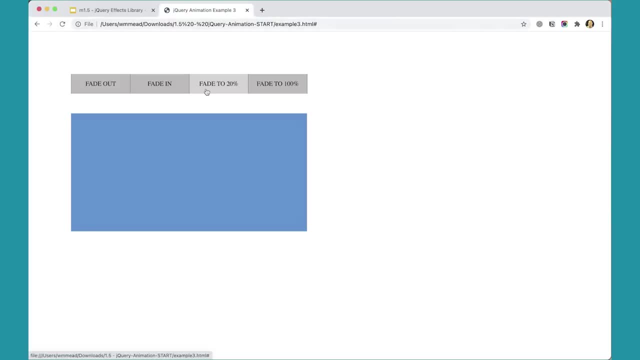 0 is completely transparent, 1 is completely opaque, and that should work just fine, so let's give it a try over here. refresh: I can fade down to 20%, and then I can fade up to 100%, or I can fade out entirely, and I can. 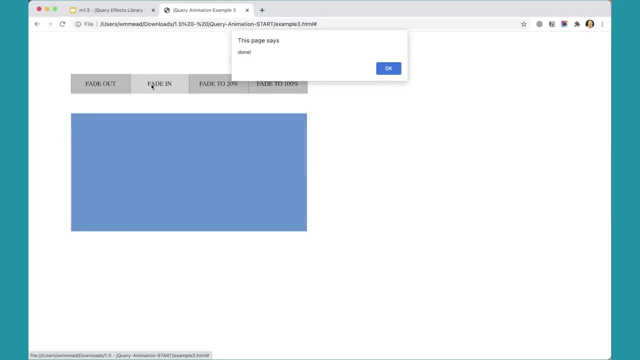 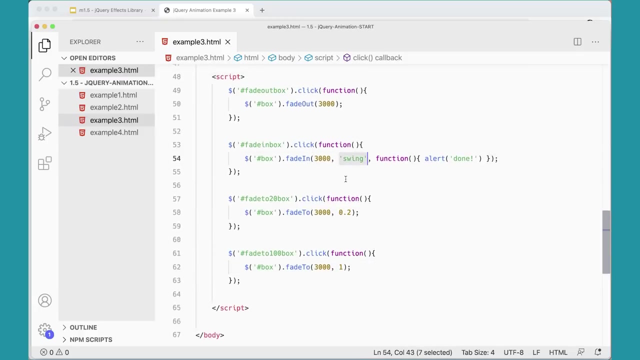 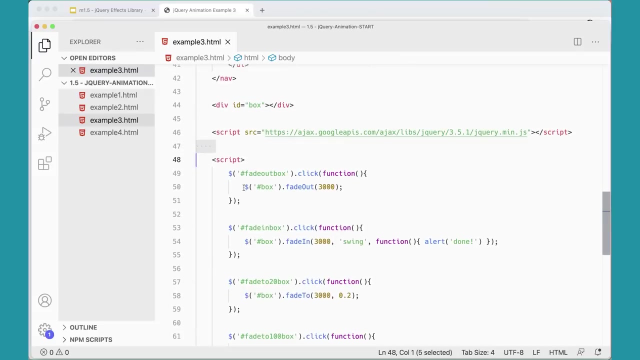 fade in entirely. so all of these buttons are working. this one has the callback function and the swing animation on it, and if you wanted to do some of the other easings, you would have to go get that easing plugin and stick it here. after jquery loads, but before we run our script. 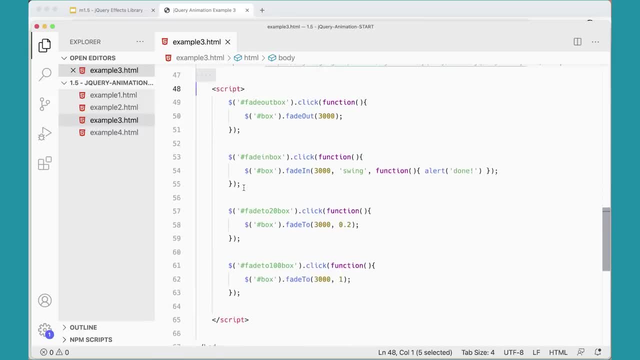 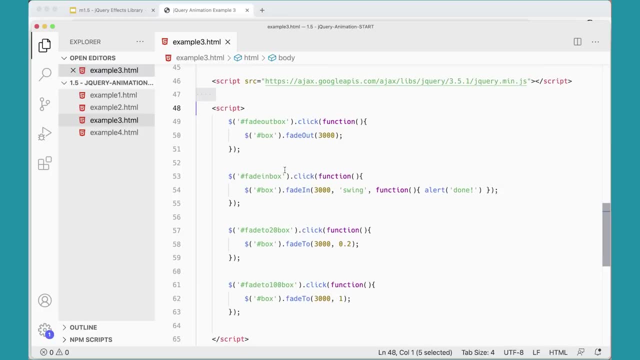 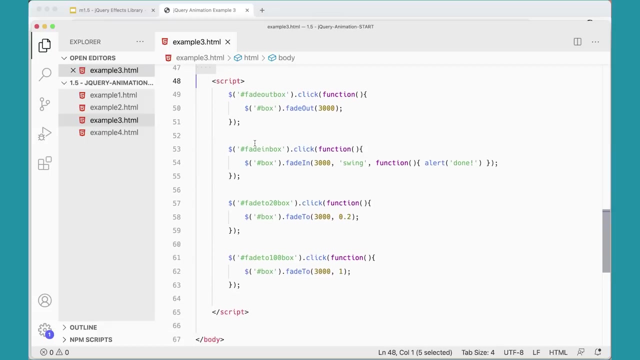 the order in which things loads matters because of the way that the functions build on each other. so we need to have jquery. in order to use jquery, we need to have the easing plugin. in order to use the easing plugin. the easing plugin has to come after jquery. 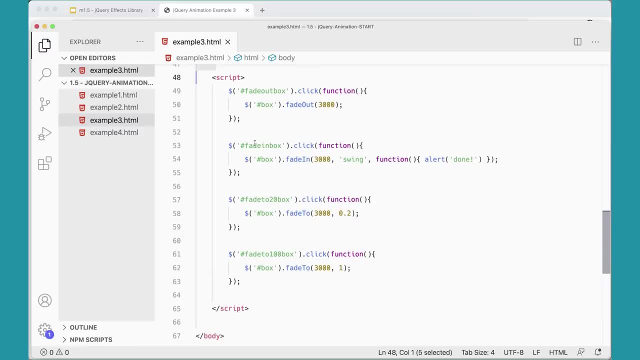 so all of this stuff has to go to work properly. we can have the callback functions and all that kind of fun stuff, and then in the next example, in example 4, we'll look at some custom animations where you can do some different kinds of things. in examples 1,, 2, and 3, 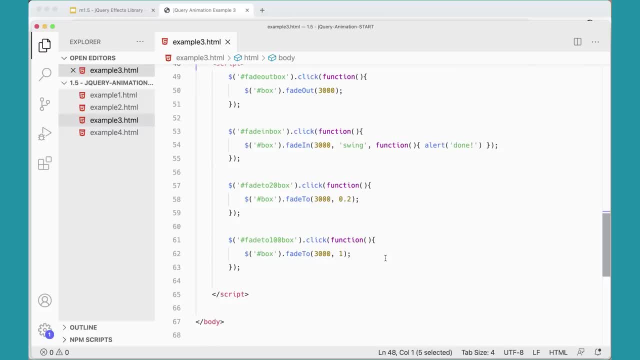 we've used some of the built in convenience functions that jquery has built into it for fading in and out, for sliding up and down, for hiding and showing and toggling slide toggle. that we commonly need to do, but sometimes you need to do a custom function. 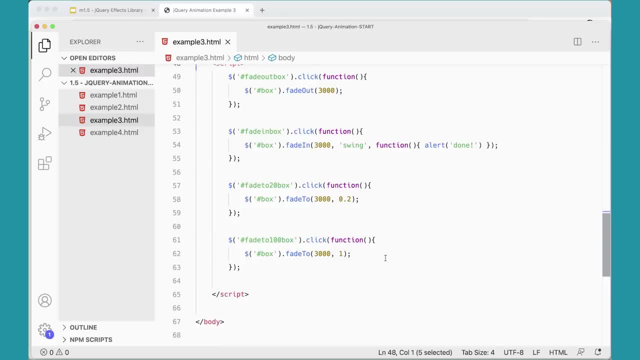 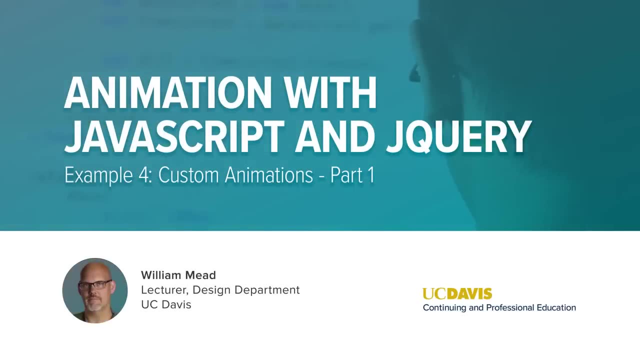 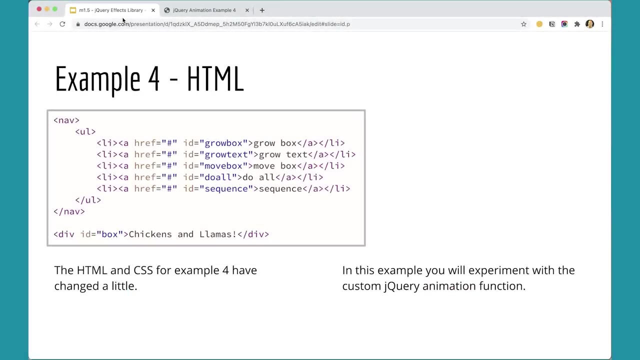 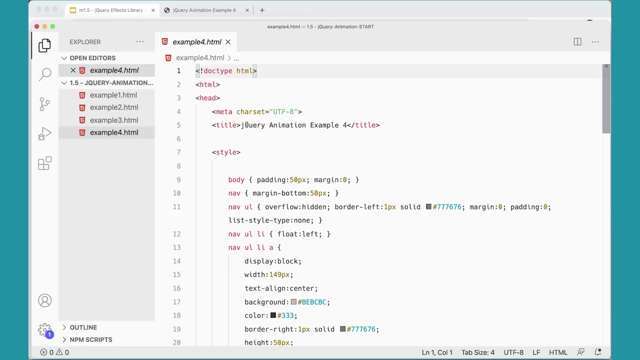 and we'll take a look at that in the next part of this lesson. next, for example 4: we're going to look at some of the custom animations you can use in jquery, and so over here I have my example 4 file open and you'll notice that. 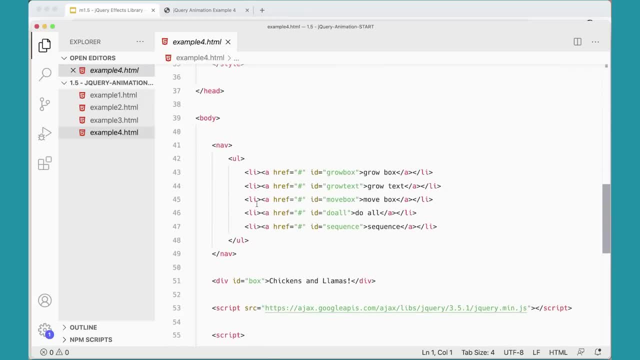 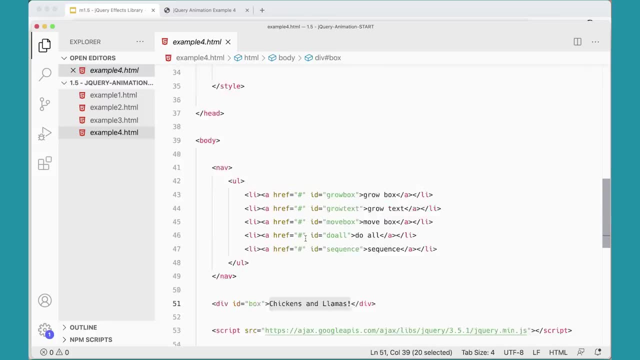 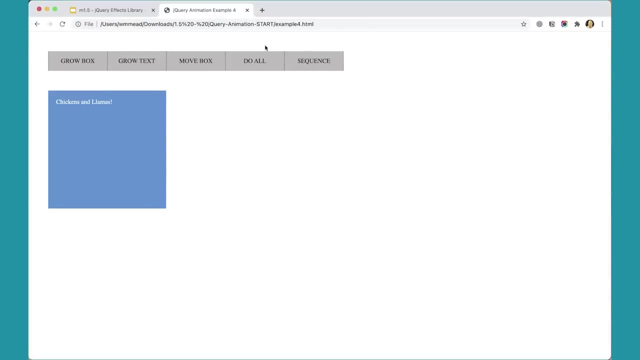 the HTML and the CSS have changed just a little bit, got more links here and my box now has some content inside the div box here and you'll see that my styling is a little bit different up here. if you look at the actual page, it looks like this now: 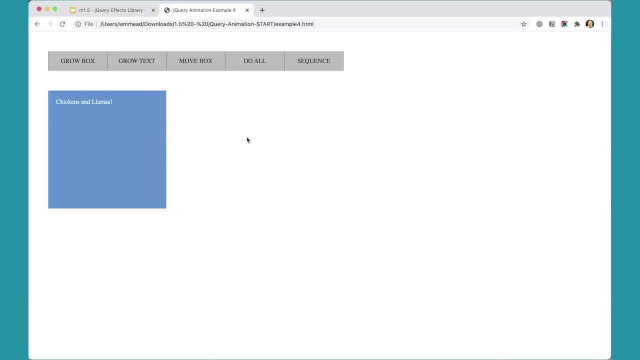 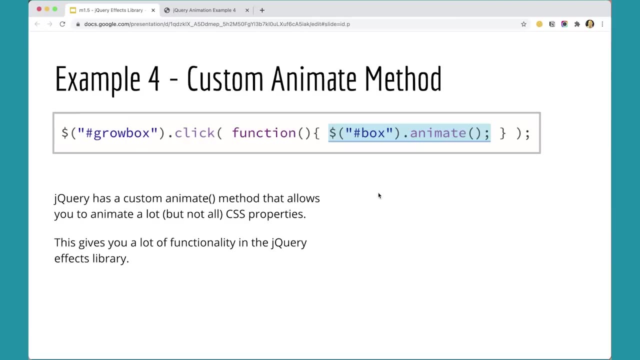 and we're going to make each of these buttons work so we can see how some custom animations work in jquery. so to do this, we'll use the animate method in jquery and you'll see that it allows us to animate some- not all, but some- of the 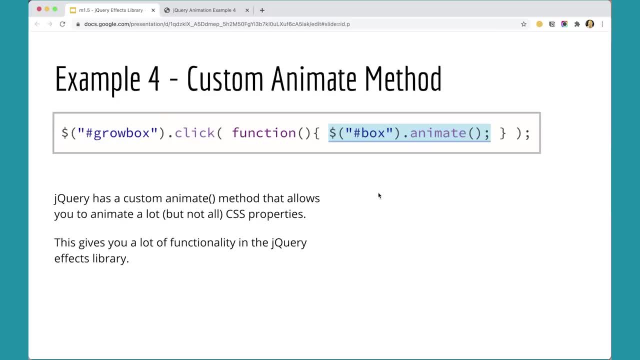 CSS properties that we have come to know and love over the years working with CSS and that gives us a lot of power, because we can actually use these CSS properties to animate all different kinds of things, not just sliding up and down or showing and hiding and doing this kind of stuff. 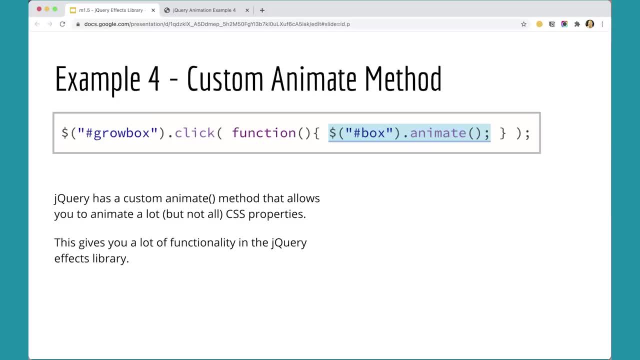 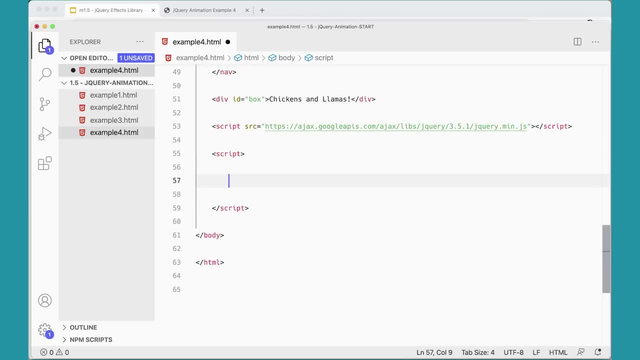 so that's pretty cool. so let's give it a try and see what it does over here. so down here I'm going to add in my script, I'm going to go get my jquery object and I'm going to get this first link up here: grow box. 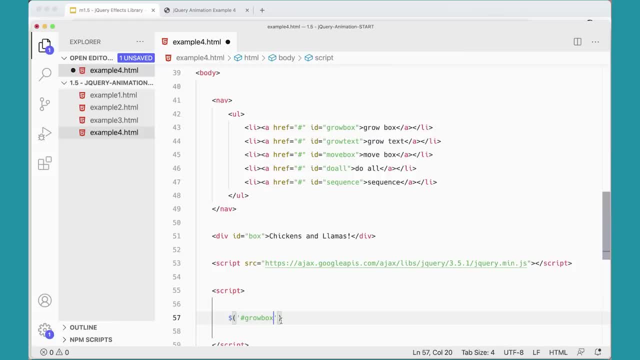 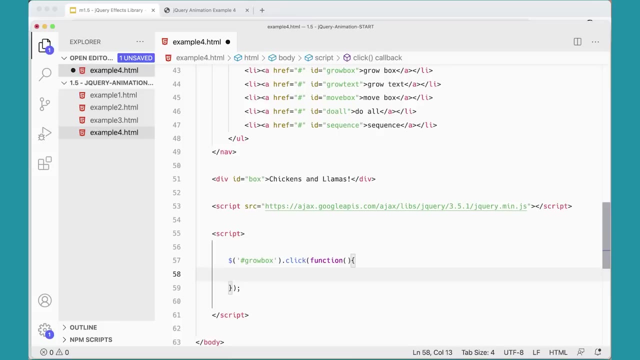 pound grow box and I'm going to add a click event handler on there and then I'm going to pass in a function that runs when you click it and everything is going to go inside these curly braces here and at this point I want to effect box. 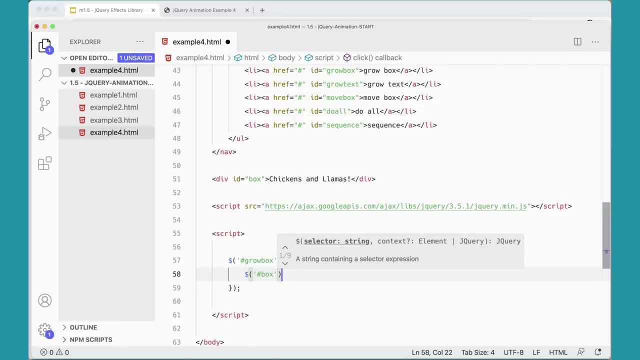 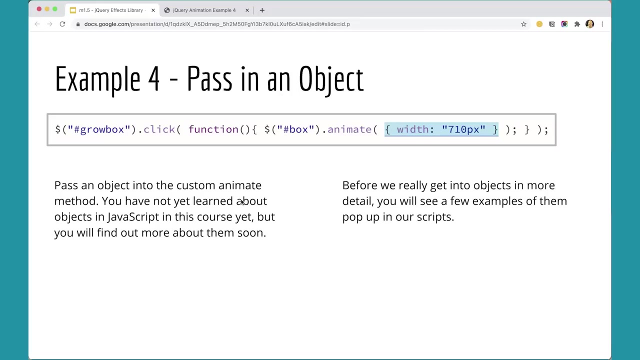 pound box. don't forget the pound sign. and we're going to do the animate function in jquery, so this will animate the the box. and the way we're going to do this here is: we're going to pass in a. we're going to pass in an object. 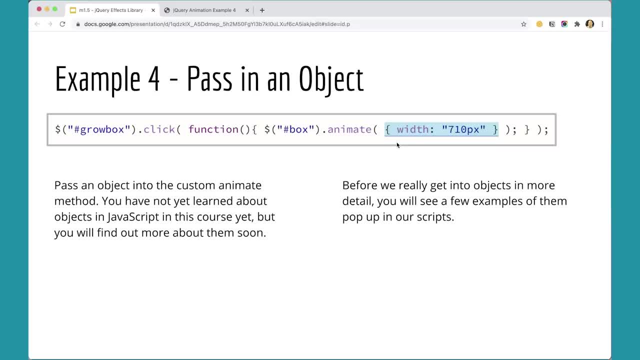 and we have not yet worked with objects in javascript. they're coming- we're going to get to them later in our instruction about javascript, but we'll see them pop up a few times, and this is one of those times, so I'll explain it just a little bit now. 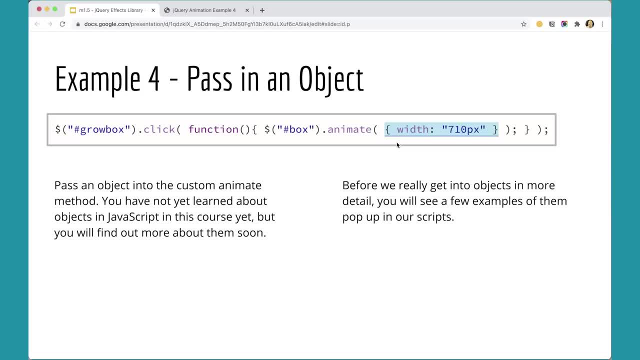 but we'll get into objects in more detail a bit later. and an object is just an alternative way of storing data in javascript and it comes with a key value pair. so we define an object with the curly braces and then we have a key value pair. so in this case, 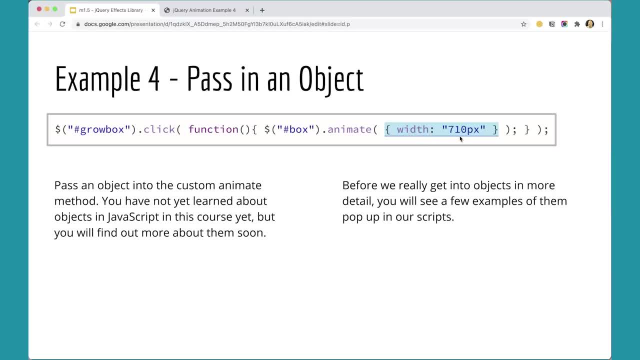 the key is width. that's the css property we're animating, and then the value is 710px, and you'll notice that the value goes inside quotes but the key does not, okay, so that's kind of a distinguishing aspect of objects in javascript in general and also in jquery. 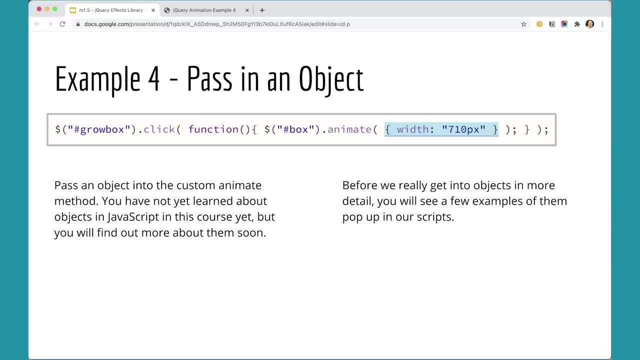 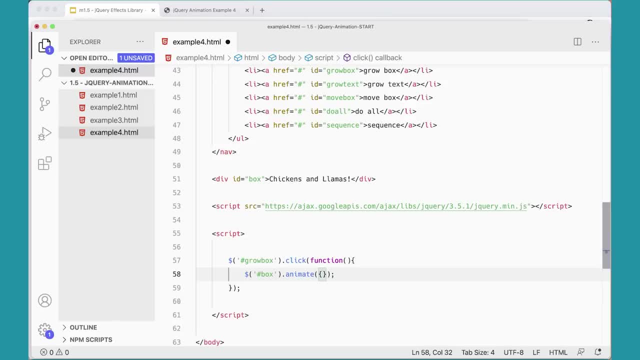 so let's go ahead and give this a try. we're going to animate in here, we're going to pass in an object open and close in curly brace and we're going to put in width colon and then in quotes 710px, and that will move the box. 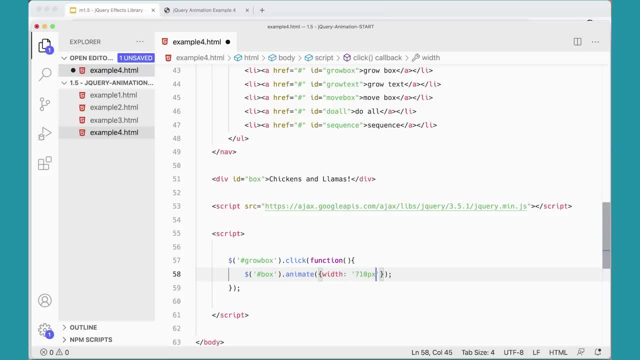 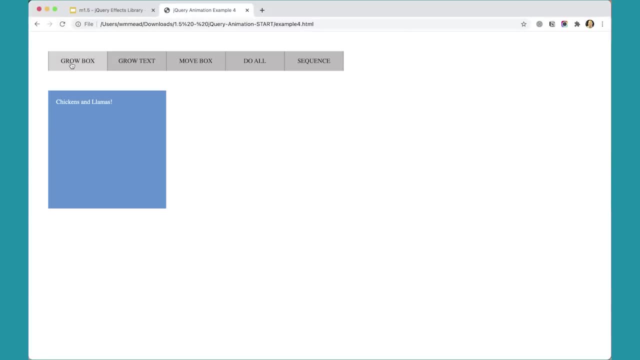 or it will change the width of the box to 710px. so let's give that a try. if we come over here and test this refresh grow box and you can see, it sets it so that it's 710px, and i knew it was 710px to end. 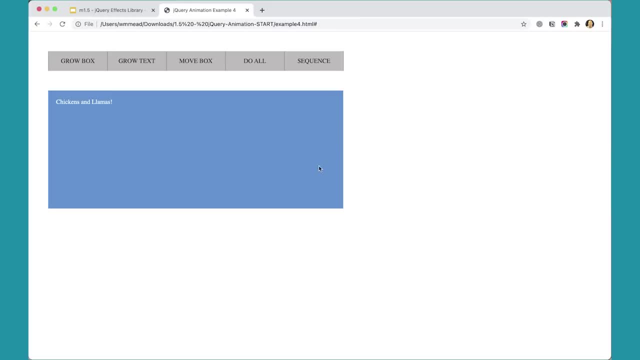 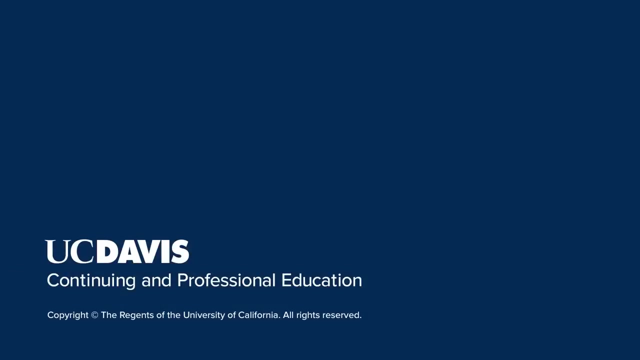 right here, so it all lines up and looks nice. so that's kind of cool. alright, so we were able to pass that in and do that one. let's take a look at the growing the text and affecting the actual text inside the box in the next video. 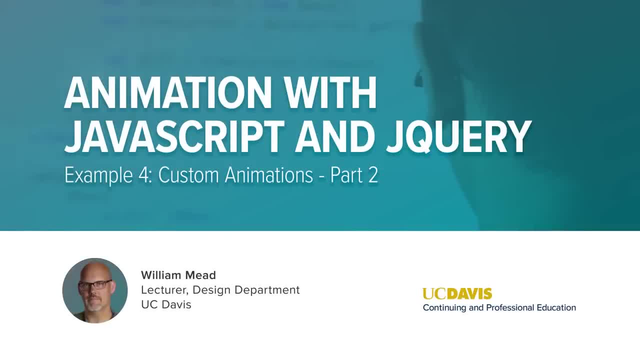 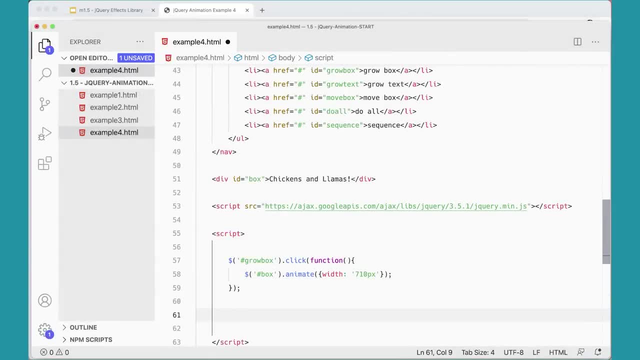 for this next example, we will start with our jQuery object again, as always, and then go and get the element that we want to get, which in this case is pound grow box, because we're getting- oh no, we're growing the text more- grow text. it's always good to copy and paste. 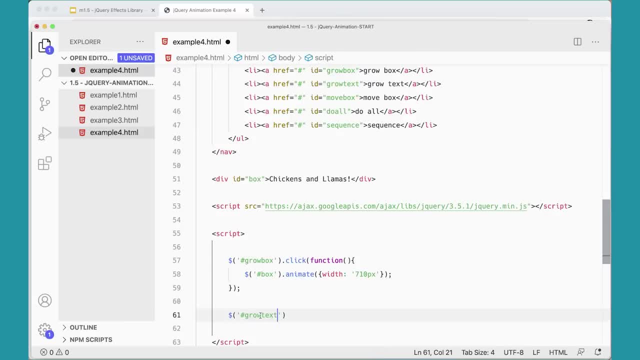 just to make sure you're getting exactly the right thing. so let's go ahead and do that, and then we'll do click parentheses and a semicolon. that click handler will run when we click on grow text. and then we're going to come in here, we'll add our function. 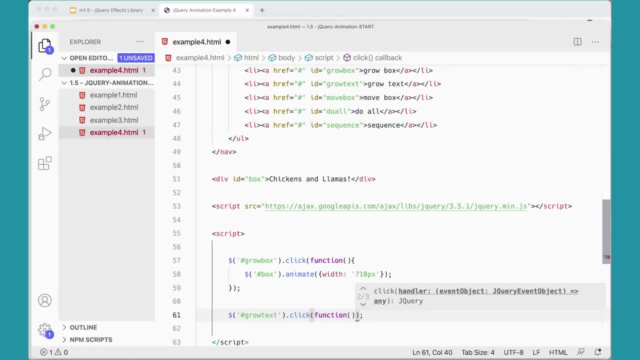 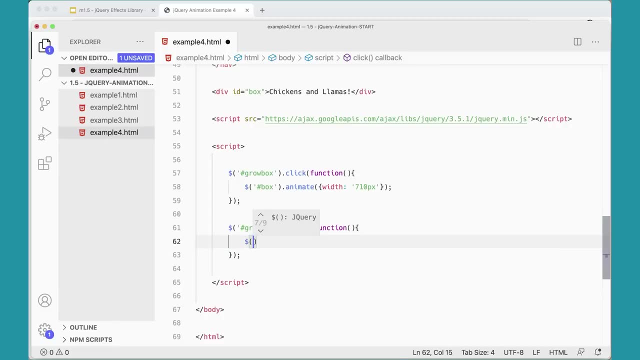 that runs when we click on that. let's put square braces, curly braces, move that down and then once again, i'm going to go get my box, pound box and side quotes there and i'm going to run the animate, the custom animate function here and again we're going to pass in. 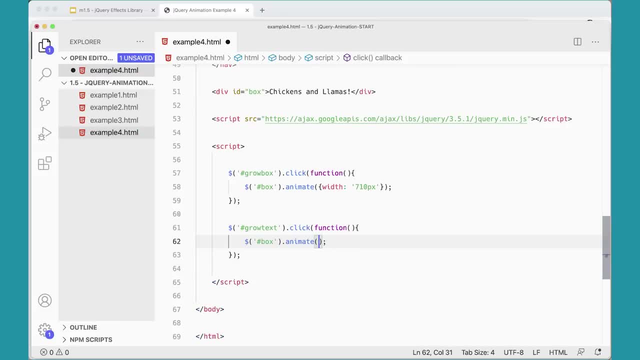 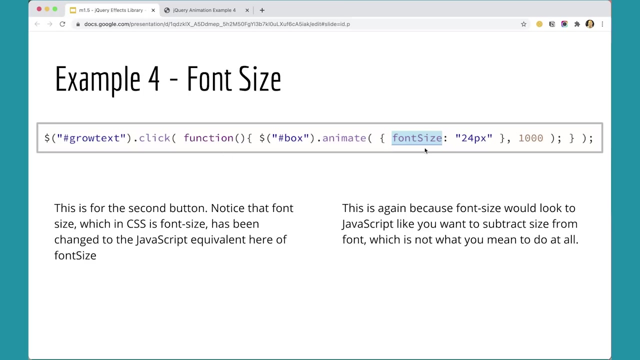 with curly braces, not square brackets. curly braces an object, and what are we going to do here? we're going to do font and quotes. now this one looks like this: come over here: font size. we're using the javascript version of font size rather than the css version. 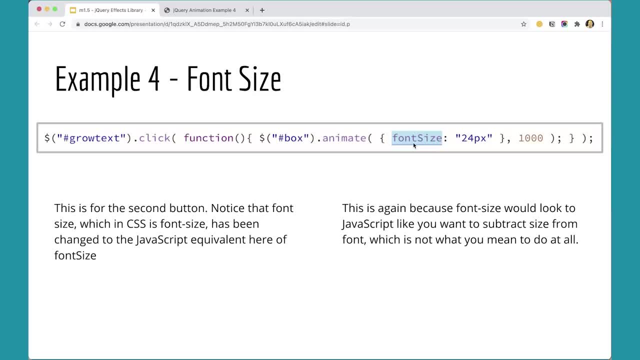 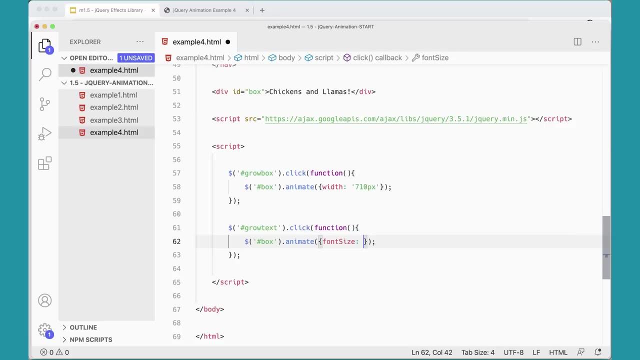 which is font dash size. so we can't have the dash in there, because javascript will think that looks like a minus sign and so it's trying to subtract size from font and that's not going to work. so instead, what we want is font size colon, and then i can set it to. 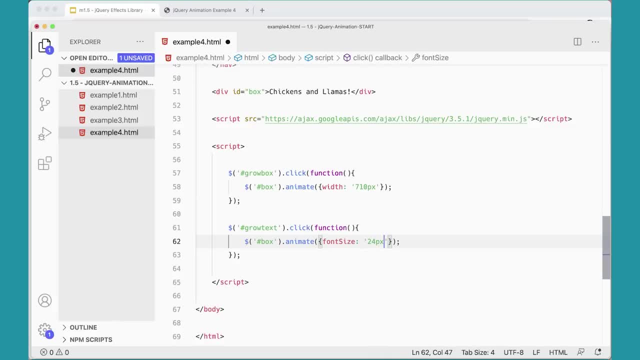 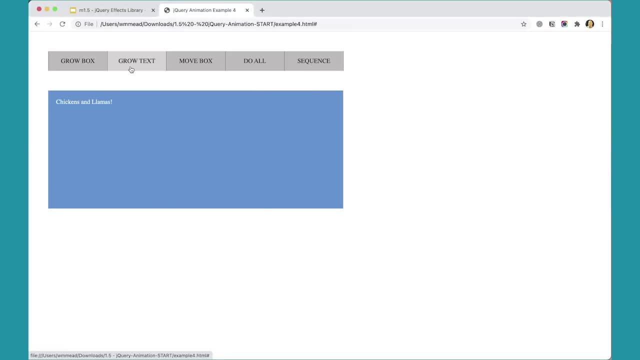 say 24px or something like that font size. so let's give it a try over here. i can grow the box and i can grow the text. whoops, did i do something wrong? maybe i did inspect console, maybe i just forgot to refresh. grow the box. 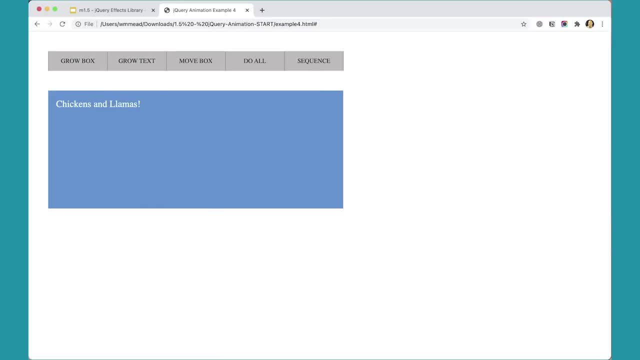 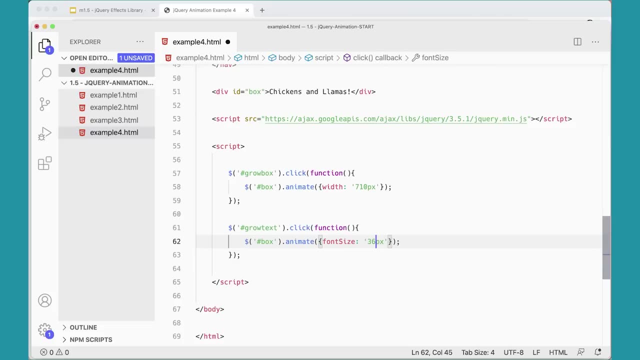 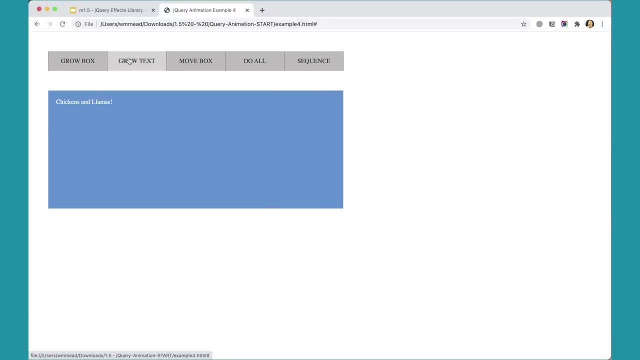 grow the text. there we go. so that's working just fine, and you can try a different size text- 40 or whatever you want to do. that would be a little bit more dramatic. grow the box, grow the text, and that's working great. ok, cool, and we could also move the box. 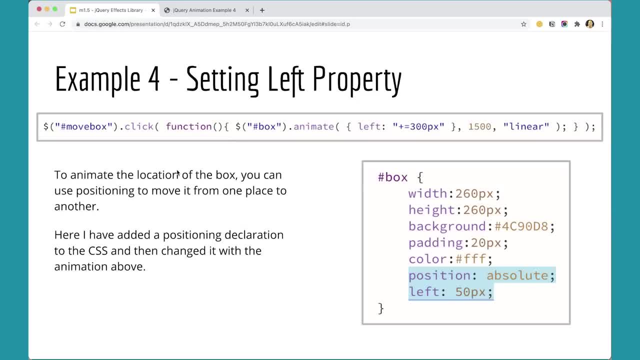 let's give that one a try. so with move box, what we're going to do is we're actually going to change the position of the box, and in order to do that, we need to set some positioning for box. so i'm going to press over here. 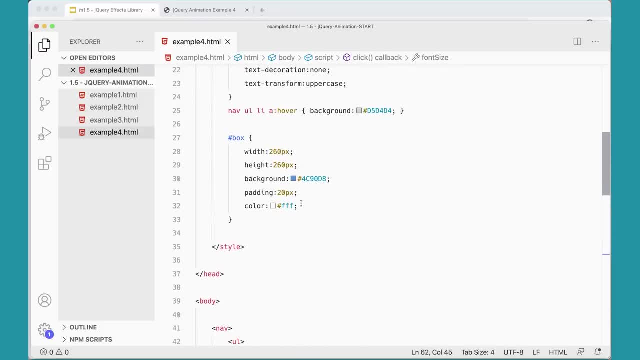 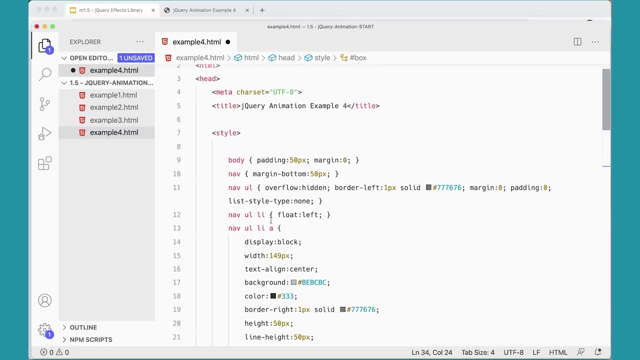 for box we need to add position absolute and then we want to set the left position left 50px. and why is it 50px? because everything else is is indented 50px in here. i think i have that padding 50px if i don't set left 50px. 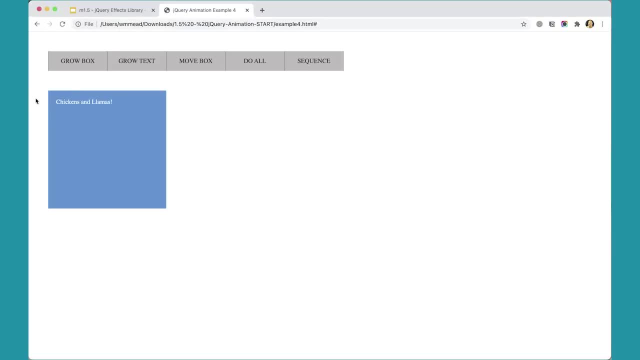 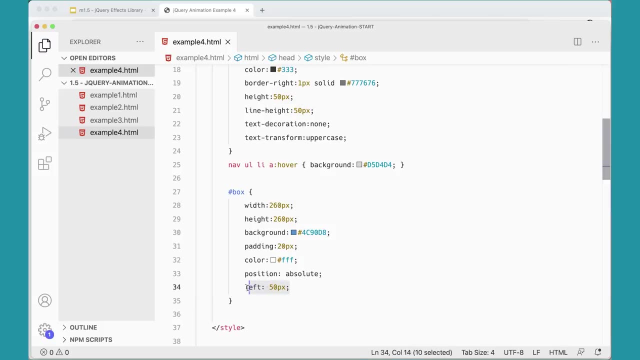 let's take a look at this really quickly. so if i reset that, that puts that in the right place, but if i didn't put the 50px in there- left 50px- well, maybe it won't actually do anything. i think that option maybe be fine. 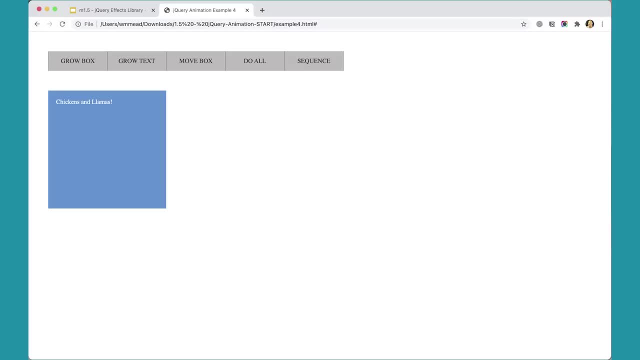 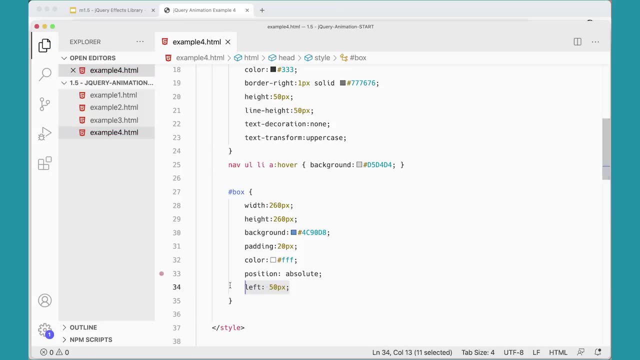 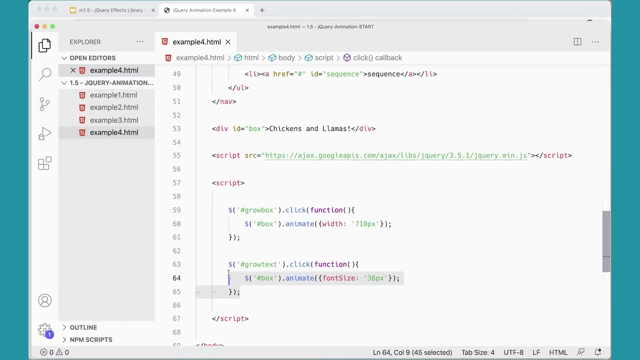 but still, i want to set the left to 50px, so that i'm- so that i'm moving from this position left 50px, because we're going to change the left property when we move the box. so down here again, i'm just going to copy this for the sake of: 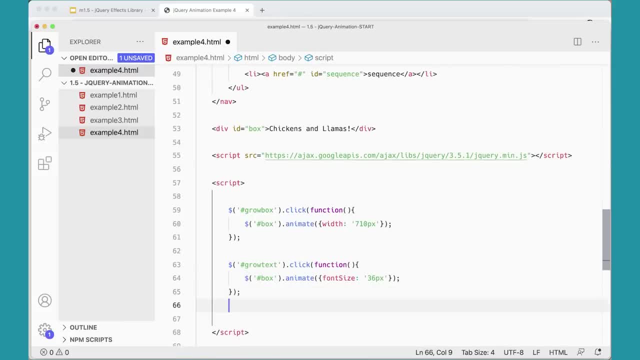 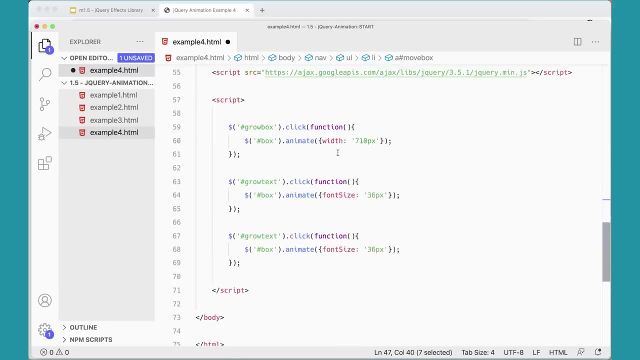 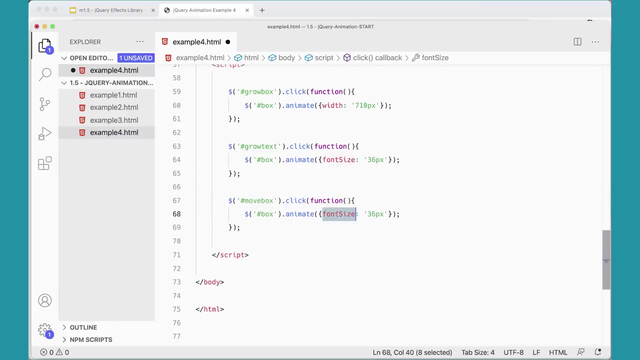 making it a little bit quicker, and down here, instead of grow text, i'm going to move box, move box, animate. and then here i'm going to change the left property left, and i'm going to do, and then here i'm going to do: plus equals, plus equals. 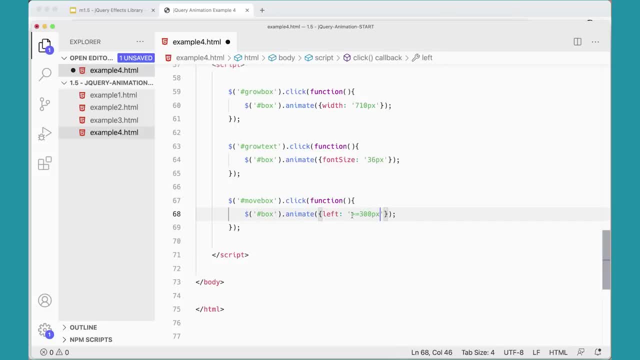 300px. so that will add 300px to the 50px that's already there, to the 50px that's already there. so plus equals will add 300px to the 50px that's already there and it will move it left 50px. 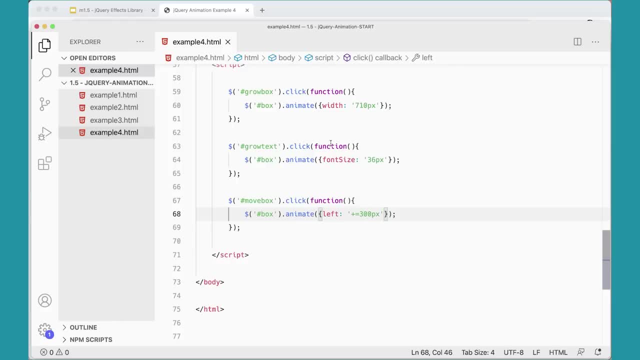 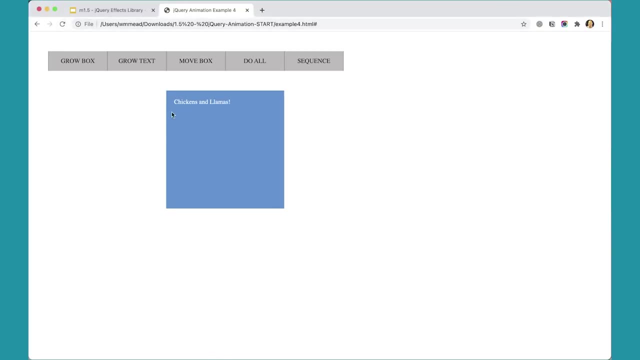 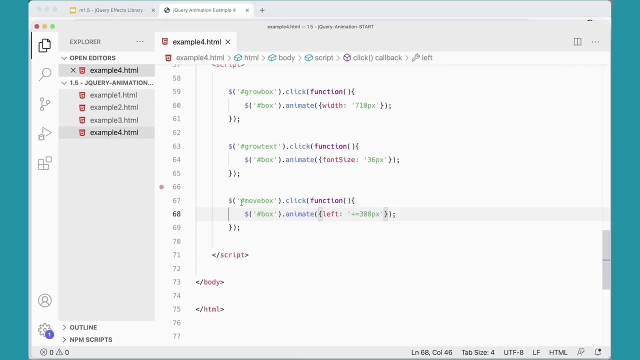 i mean to 350px. i mean to 350px from the left hand side. let's see if that works. so i'm going to move box and look at that, it moves it exactly where i wanted it to go and that's really cool. so you can set how long you want that animation to take. 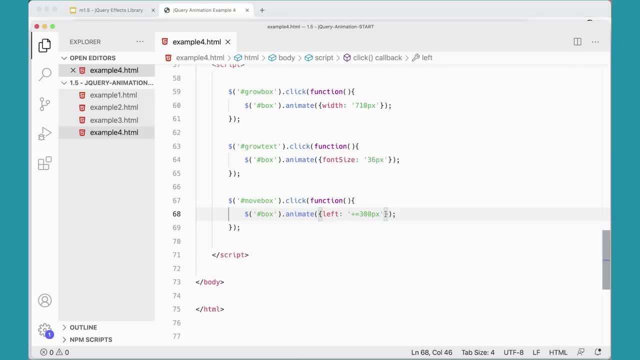 you can make it go longer if you wanted to. after the animate, after the object here, i could add in a comma and say i want this to run over 5 seconds, something like that, and that will animate over 5 seconds. so let's see what that does. 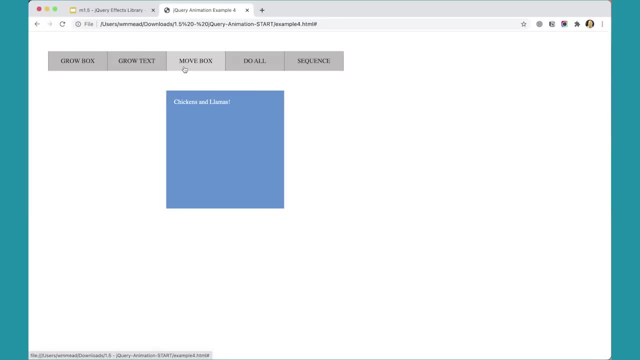 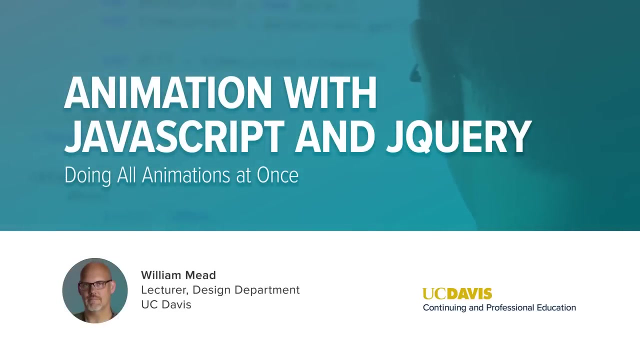 5 seconds is really slow, but it is animating it and that's pretty cool. ok, great, so we're able to adjust the amount of time and the amount that it moves and what it does with the actual animation. all with custom animation for our next button. 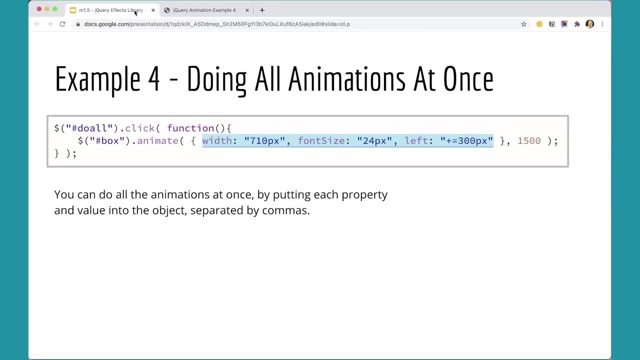 on example 4, we want to actually make all of these animations happen at the same time, so they're all going to move forward at the same time. so we will change both the width, the font and the left positioning- all three of these. we're going to change all of them at once. 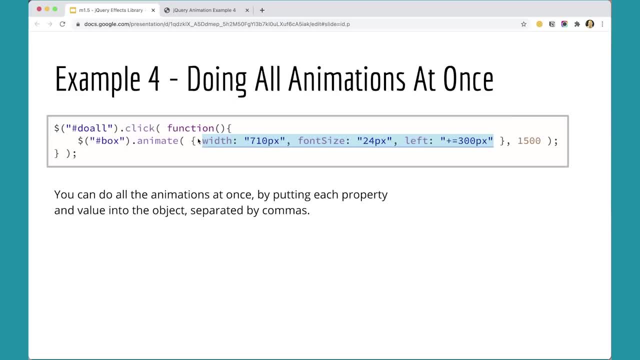 and we can do that by just passing in these different properties into our object all at once, separating them with commas. so let's go ahead and do that, because that's pretty interesting to be able to see that actually work so down here. once again, i'm going to use my jquery. 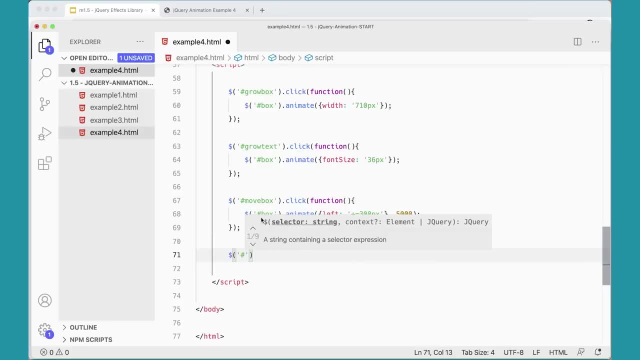 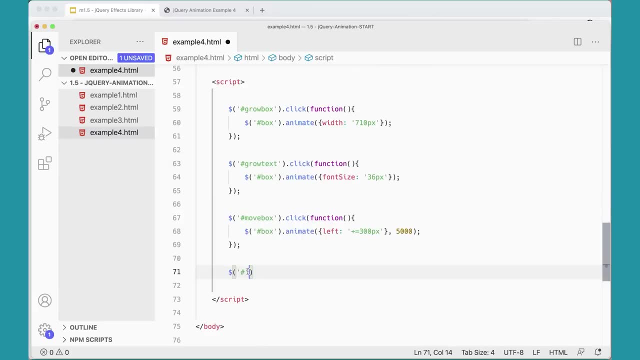 object to go get this pound, but what i want is do all, do all. so i'm going to get pound, do all, and then i'm going to add a click handler- click for when you click the do all button, and then we're going to run a function. 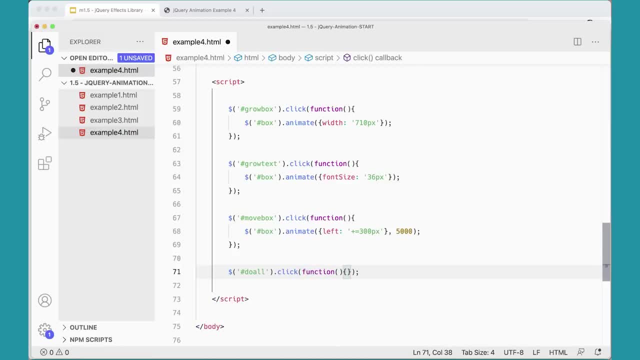 when that button is clicked, and there we have it. so here now we want to effect box parentheses, pound, box, like so, and again we're going to do the animate method and we're going to pass in our object. so we do the curly braces, and first we want 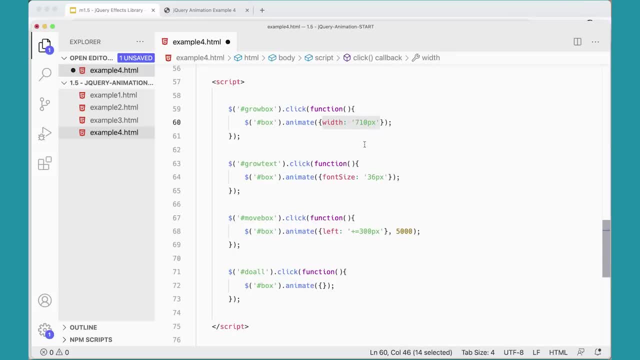 width 710 pixels. so i'll put that in here with 710 pixels and then a comma. and then we want font size 36 pixels. put that in there and then a comma, and then we want: left plus equals 300, so we'll put that in there. 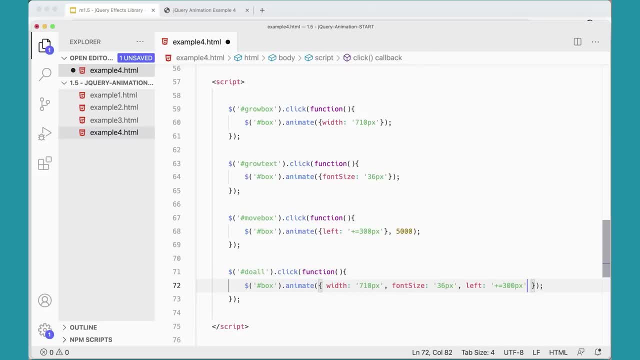 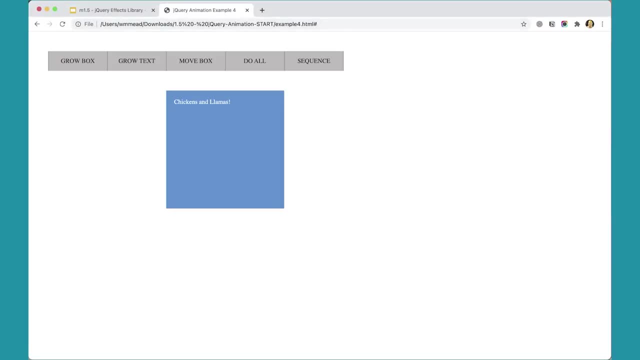 and you'll see now i've got some extra spaces at the end. it doesn't really matter, it's fine. but you'll see with all of those in there that now when i come over and test this thing first, i also want to put in an amount of time. 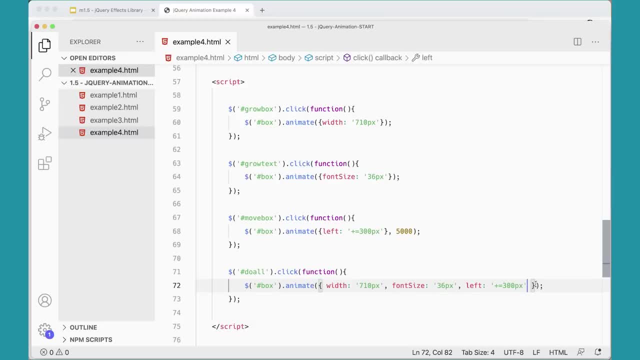 that will be really helpful. so after the curly brace, put a comma and then i'm going to put 1500. so that's going to go over a second and it's going to take a second and a half to do all of these. so let's come back over here. 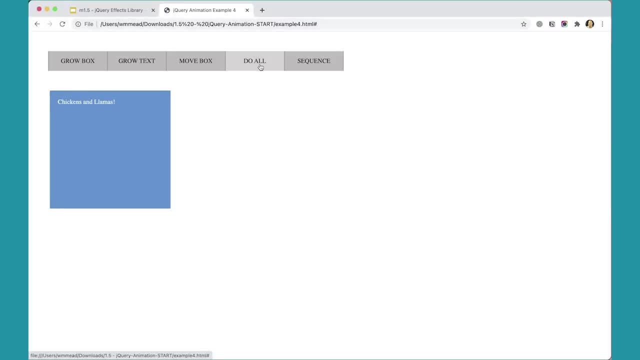 and refresh this and when i click do all, it should do all of those things. pretty cool, it runs all of them at once. now the last button is to do them in a sequence. what if we want to do? first we want to grow the box, then we want to move the box. 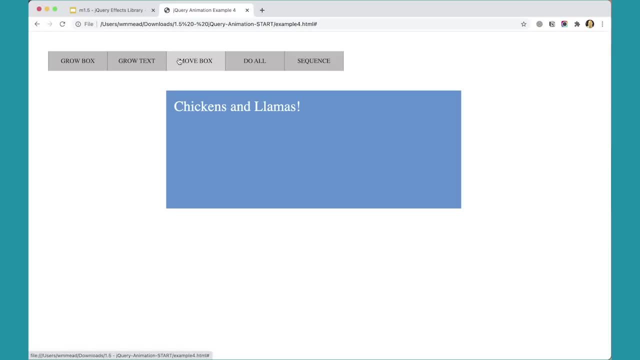 so we want to do each one of these in a sequence and we can do that with callback functions, so each one of these animations can have its own callback functions that when it finishes, it calls the next one, and when that one finishes, it calls the next one. 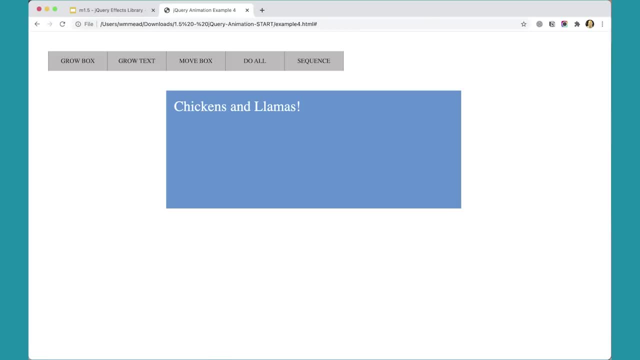 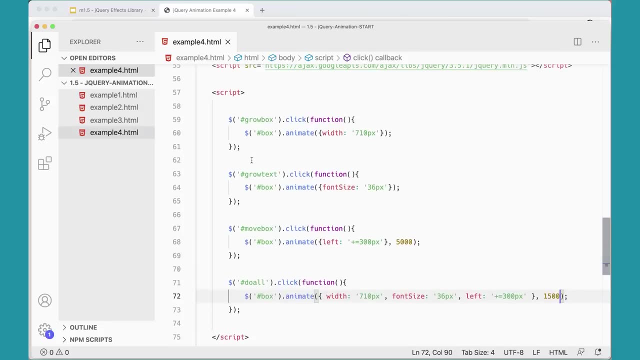 it can be confusing for the syntax in order to get this to work, but once you sort of understand it and know how to do it and mess with it a little bit, it's not too hard. so let's start with this one. i'm going to copy that: 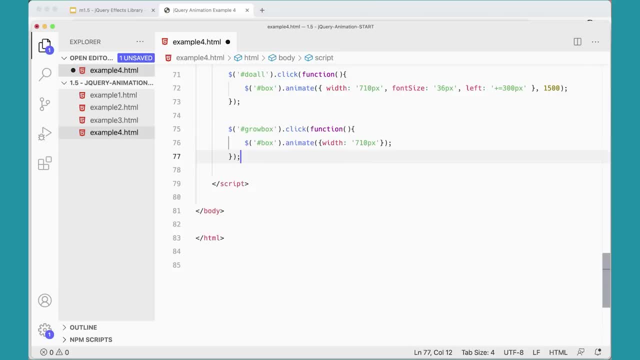 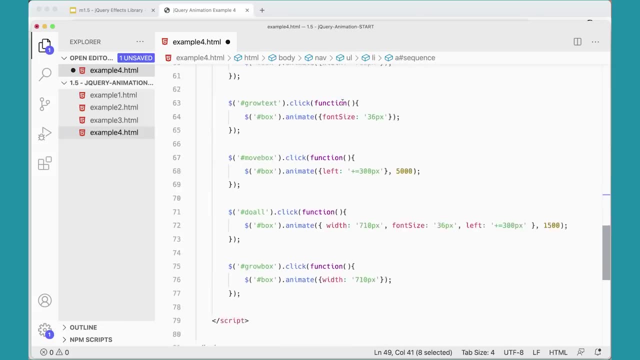 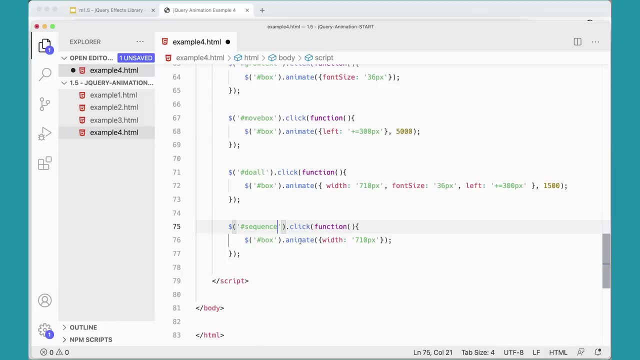 and stick it down here and instead of getting that button, i'm going to get this one sequence. so when you click the button sequence, it's going to take box and it's going to animate the width to 710px and i'm going to put a comma. 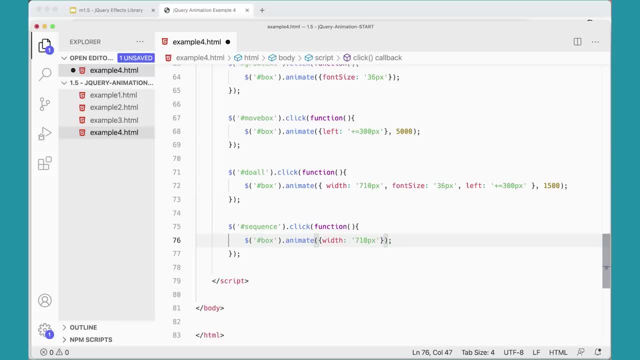 and then another comma. yeah, i'm going to put a comma and then i'm going to put, say, 1500, for how long that animation should take place, and then i'm going to put another comma and i'm going to add a function. okay, so it's really easy to get confused. 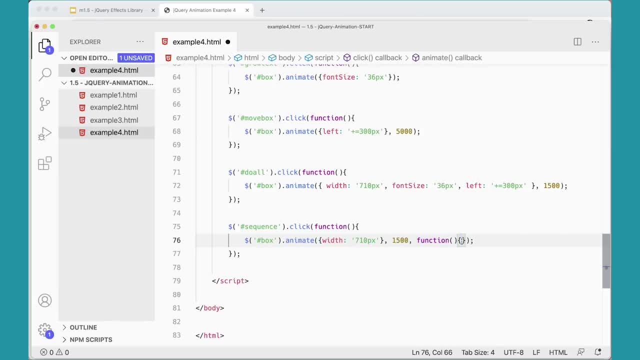 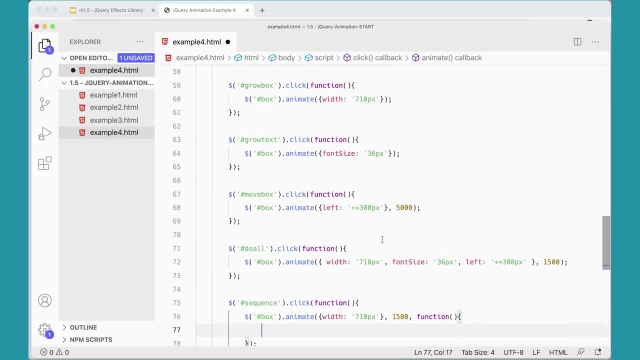 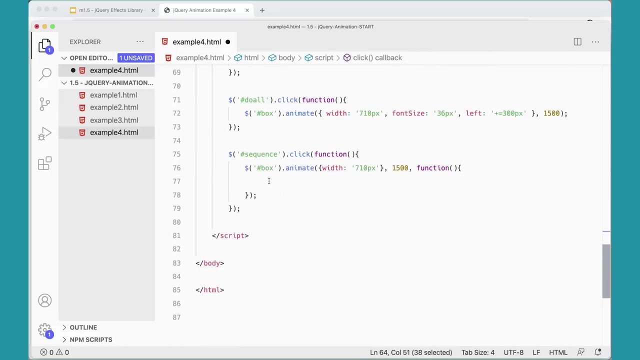 here, because we're going to put everything into this function here. so i'm going to click between those curly braces, move that down, and then i'm going to go get this one font size 36 and i'm going to put a comma here and i'm going to put 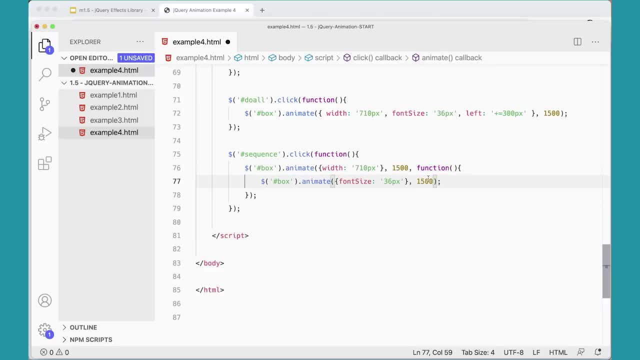 1500 seconds in there, so 1500 milliseconds, it's one and a half seconds. 1500 milliseconds in there, and then a comma and another function, parentheses, curly braces. it's really easy to lose track of this stuff, so you have to be really careful with it. 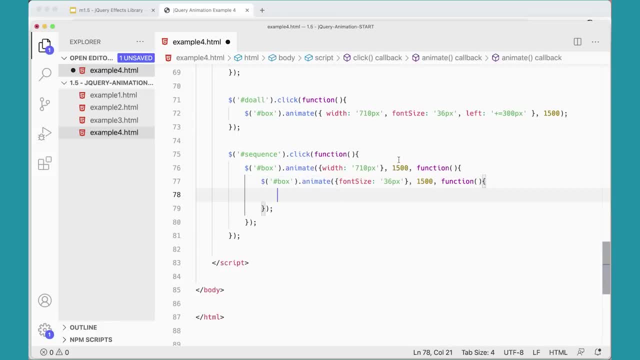 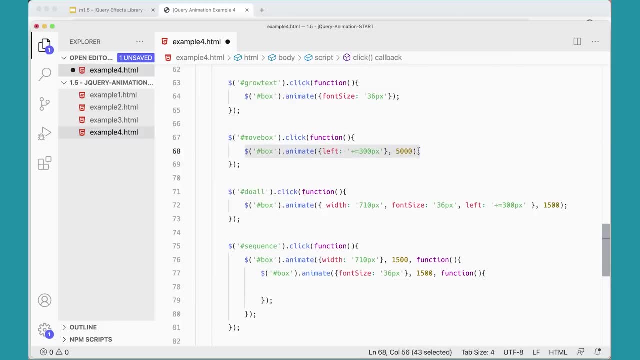 but then i'm going to put the next one inside these curly braces, so i'll move that down and i'm going to do this one here. i'll change that to 1500. there we go, and that's the last one, so it doesn't get a callback function. 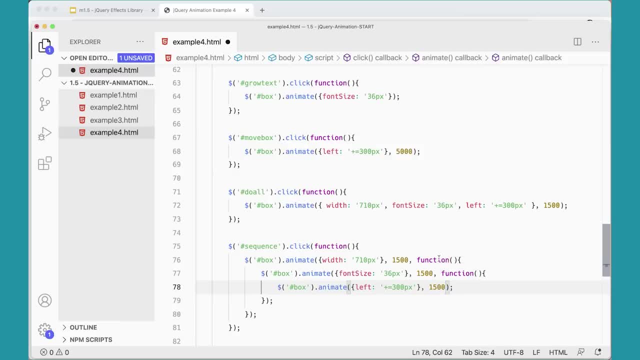 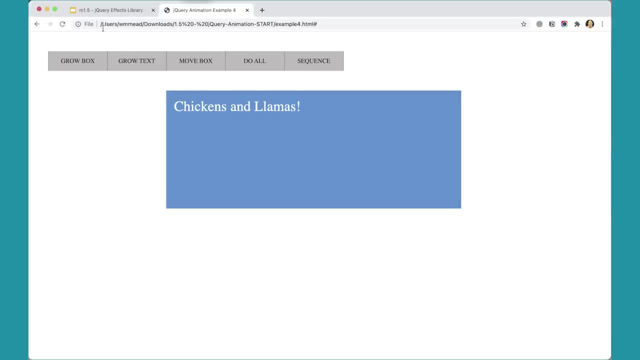 so i've got a callback function inside a callback function inside a function that happens when i click and let's see if that works. if i come over here and test this refresh, if i did it right sequence, it should do that one and that finishes. it does that. 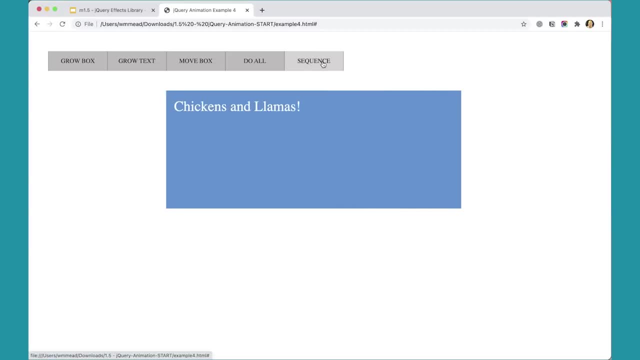 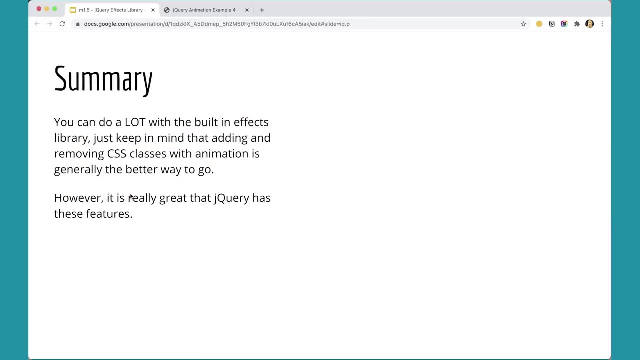 and then it moves it and everything is working well in the sequence and that's pretty cool. so with the javascript effects library we can do all kinds of really interesting things and you can animate all kinds of different css properties. however, it is better to do the animations in css. 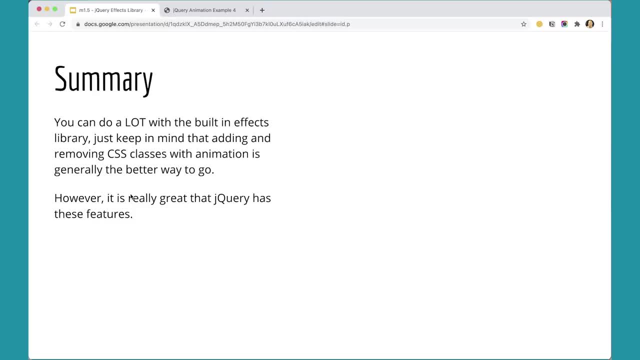 with transitions or keyframe animations in css and then apply those classes. but sometimes using the effects library in javascript is still useful and especially if you're doing something fairly quick, there's not a lot of reason not to use it. so we'll see an example of 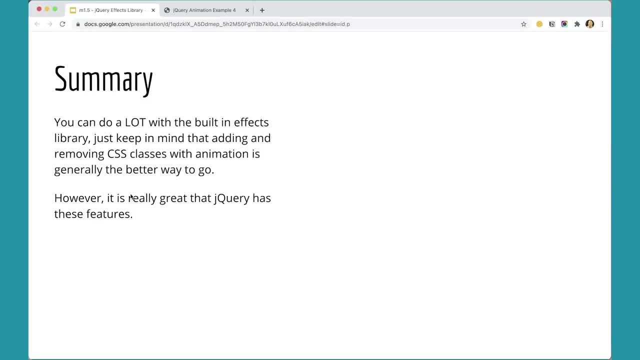 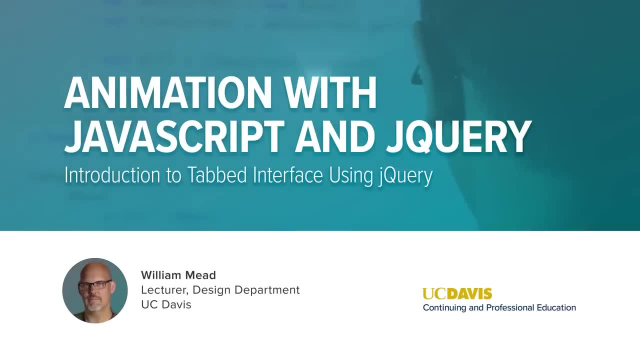 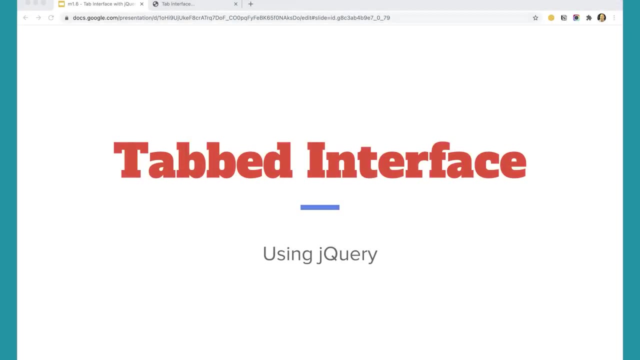 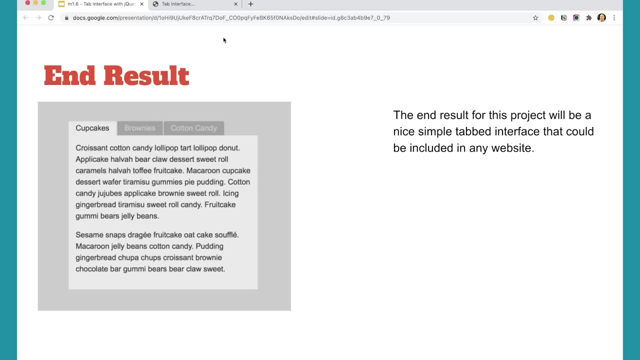 when is a good place to use this effects library coming up when we create our tabbed interface? tabbed interface, tabbed interface using jquery. we're going to create this tabbed interface and this is a really good project to see the jquery effects library in practice. 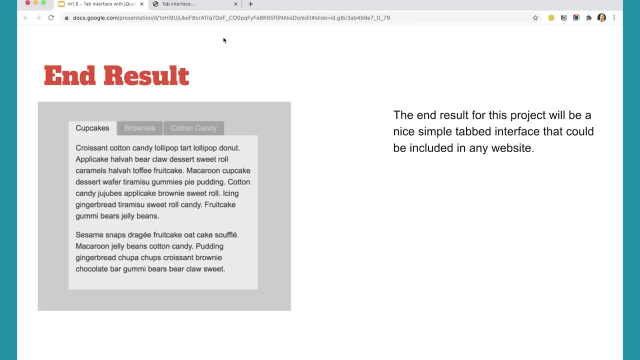 and we've looked at how to use the jquery effects library and now we're going to use it a little bit in this project and this is a really good project for seeing how that effects library can be effective without adding a lot of extra weight to a project. 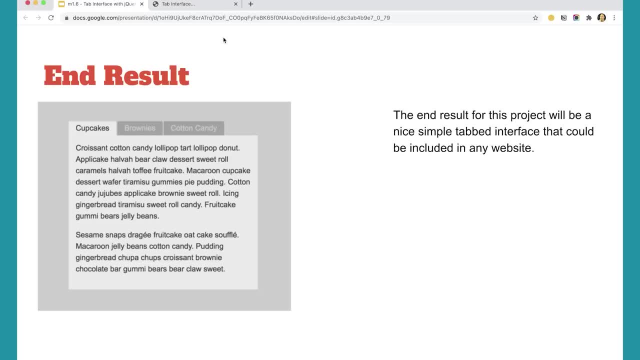 we're not going to do anything too intensive with it, but it's kind of a nice use of the effects library and then we'll actually remake the same project using plain javascript. so you can see the difference between the two. compare the code between the two versions. 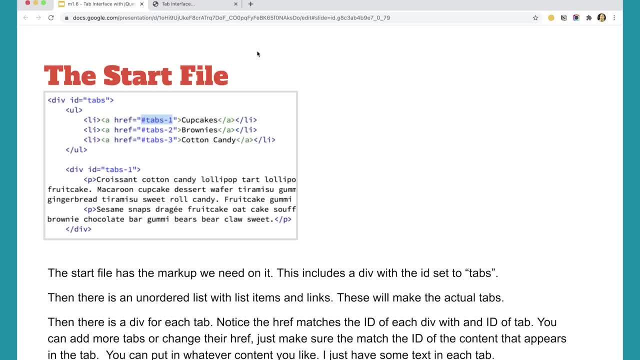 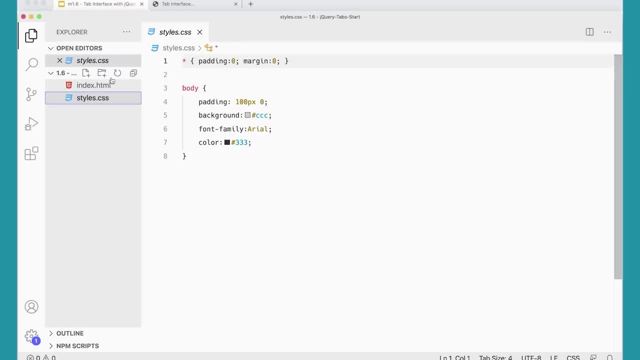 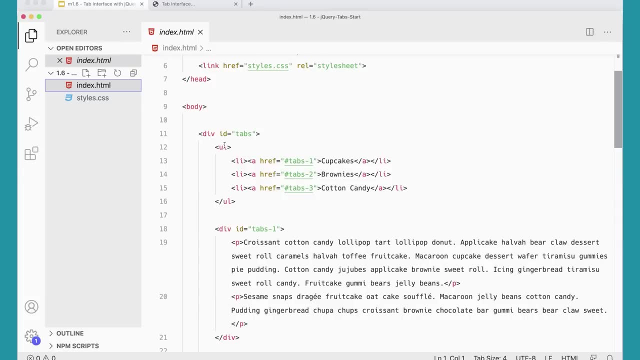 so let's get started and see what this is going to look like. if we go and look at the markup file over here, you'll see that we basically the way it's set up is we have a div called tabs, with an id of tabs, and in here we have an unordered list. 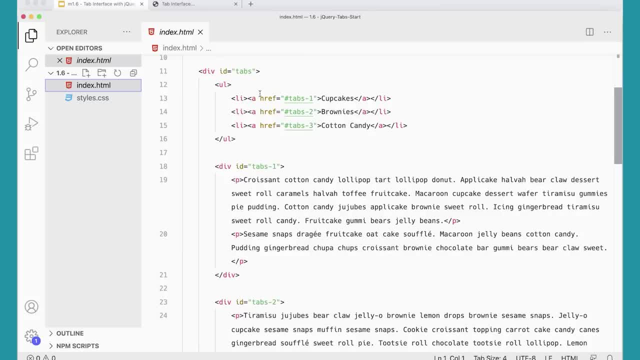 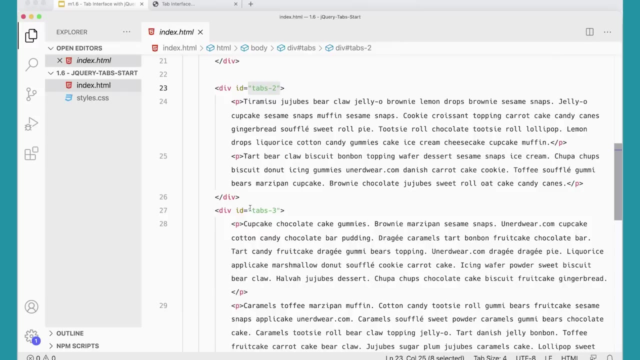 and these things are going to be the actual tabs that you click on and then the href for these links to the ids for these pieces of content down here that will be on each tab, and this is typical for the setup for this type of interface. is that you would have? 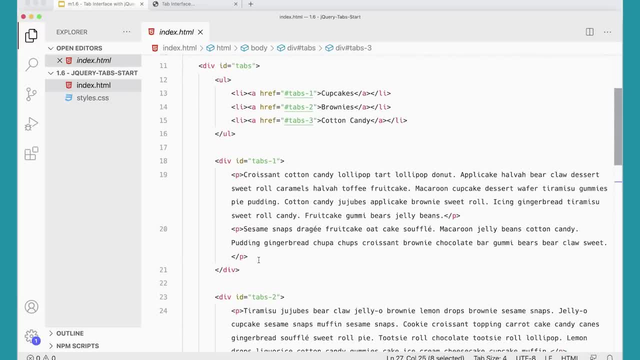 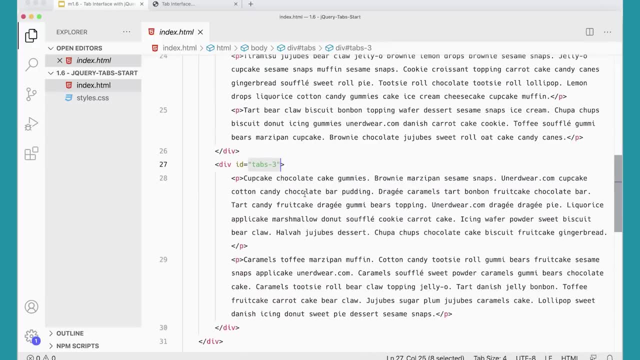 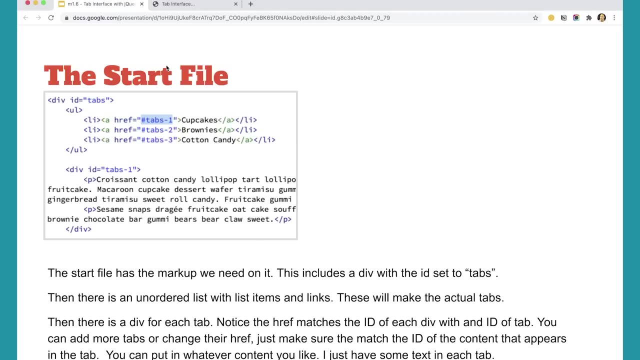 an unordered list that makes the tabs, and then the tabs themselves would have ids that match the hrefs for them up here. so that's the basic markup that we're going to be using and it should really work well for us. so from there we need to add: 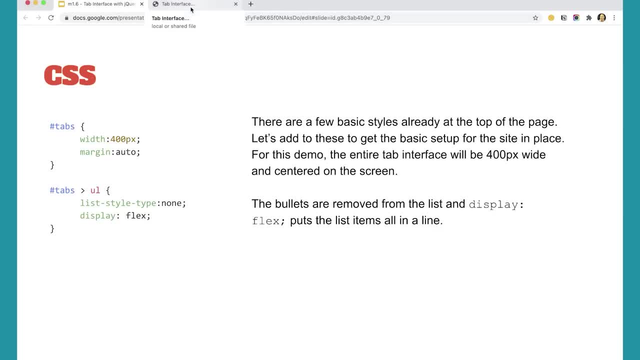 some basic styling because currently the page, if you open up the start files in the browser, they look like this. so there's very little styling here. I've done just a tiny little bit on my style sheet so you can come over here and see in stylescss. 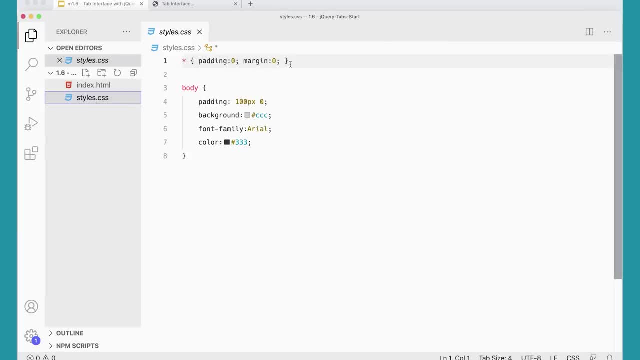 I've just got this reset rule, which is not great to use for production websites but for this. it's just taking margin and padding off of everything and then we're just adding some padding to the body and setting the background color and font color. so let's add a few rules here to 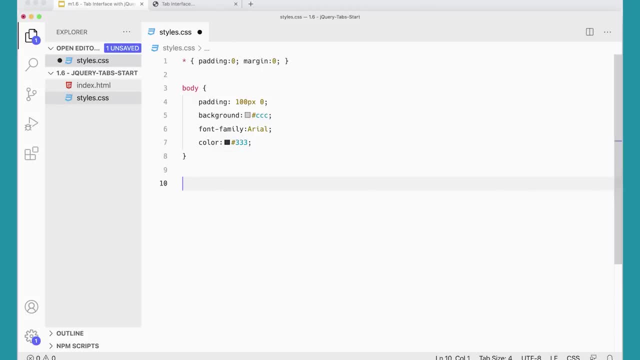 kind of make sure that we get this thing all in place. the first rule I'm going to add is for the tabs themselves. so this is the entire interface. really, I'm just going to give it a width of 400 pixels and set margin to auto so that it centers on the screen. 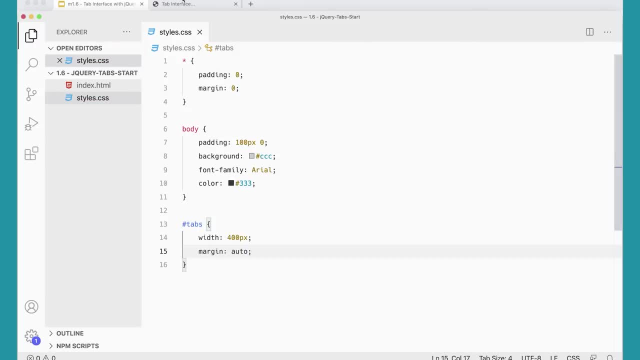 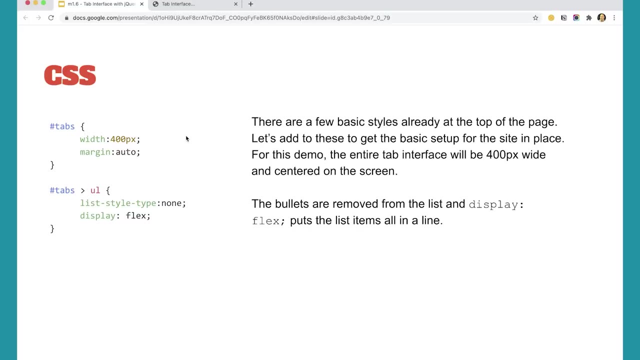 so, with those two pieces in place, you come over and refresh this and you can see now it's looking like this. so we've got that. and then for the actual tabs, for the unordered list, I'm going to get rid of the bullets and set them to display flex. 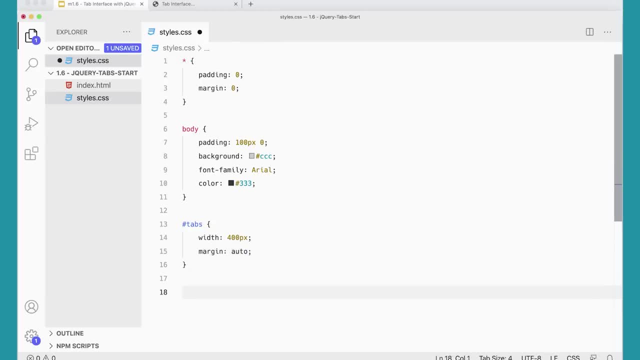 so they go next to each other. so tabs, pound tabs, angle bracket, ul- I'm going to say style type but not none, and then display flex. there we go. now you might wonder about this angle bracket in here, and when I save my file, Visual Studio got rid of my spaces. 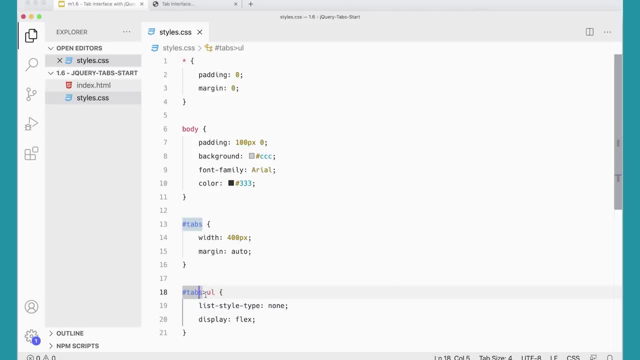 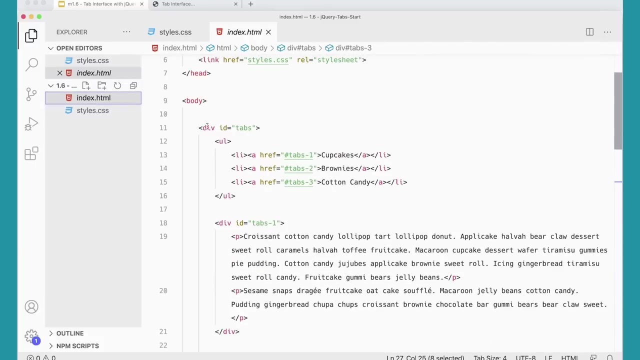 I kind of like the spaces in there. but you might wonder about this angle bracket, and what this does is it makes sure the ul, the unordered list that's inside the tabs- directly the direct descendant, is targeted, so in other words the only unordered list that would be selected. 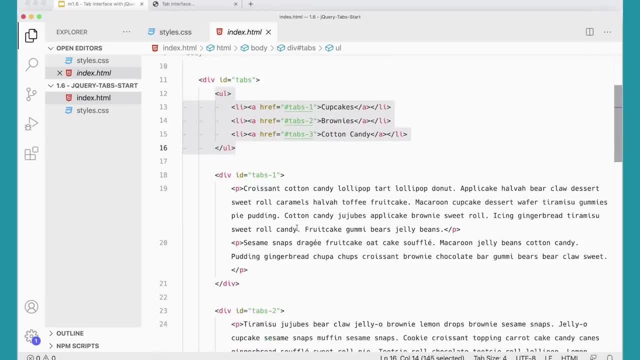 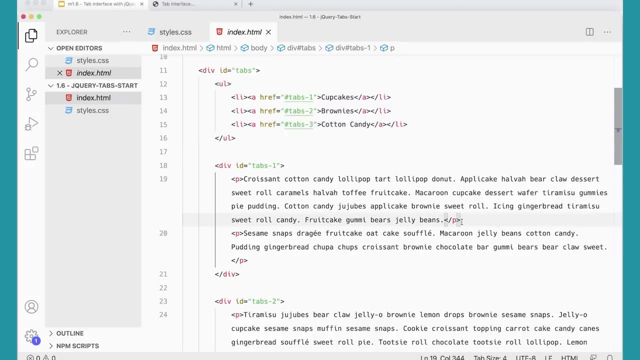 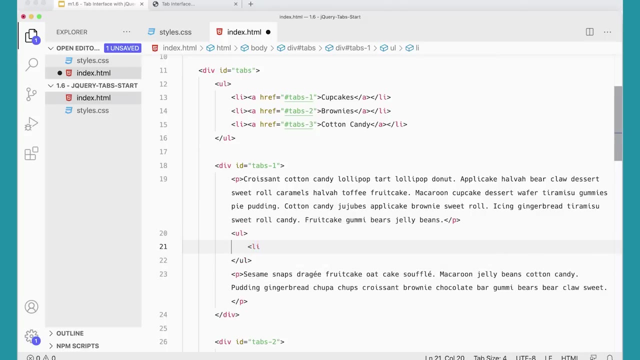 is an unordered list that's a direct descendant or direct child of tabs. it's possible that inside my tab content here maybe I'd want to have an unordered list of things. I might want a ul with, you know, with some list items. example one: something like this: 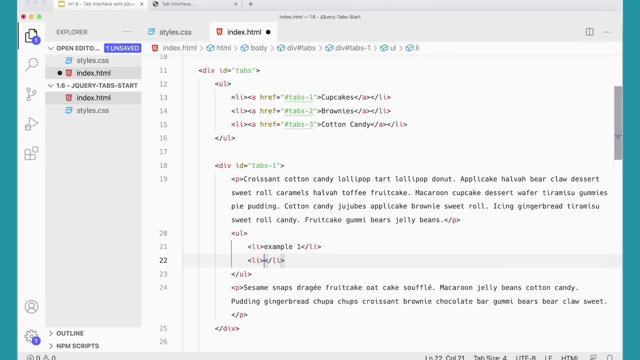 li. example two: I don't know something like that, but I don't want this unordered list to get targeted by my rules. I only want this one, because this is actual content in my tab, so that's why I'm using the angle bracket here- is that it will only target. 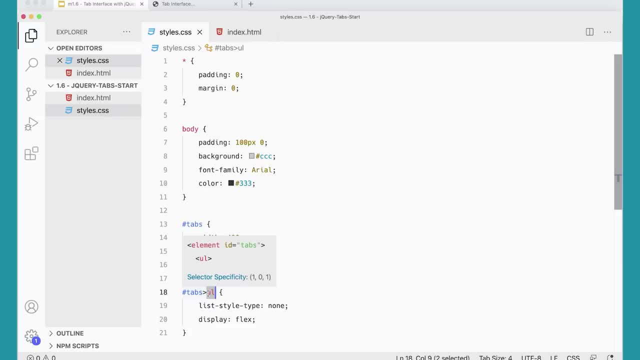 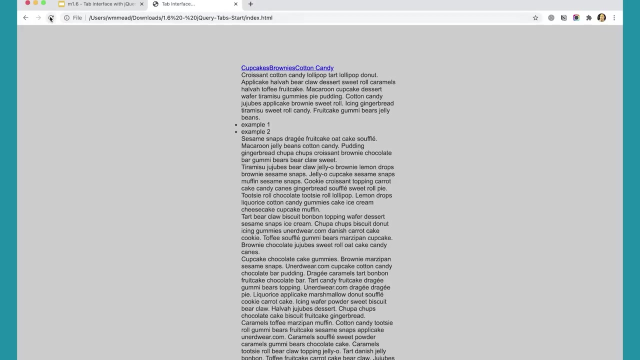 the specific selector for my element tabs that you have there. so that will actually work for that. alright, great, so we've got that in place and now my tabs are lining up next to each other. still doesn't look very good, but we're getting there, ok, great. 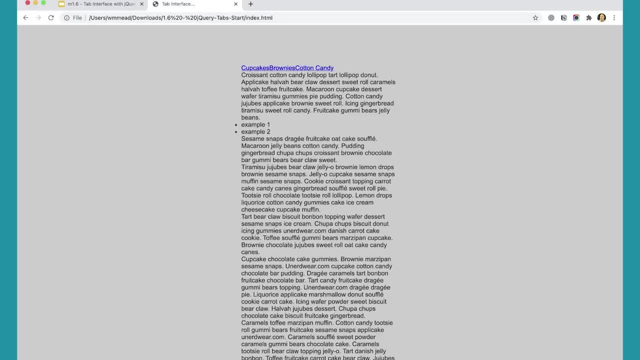 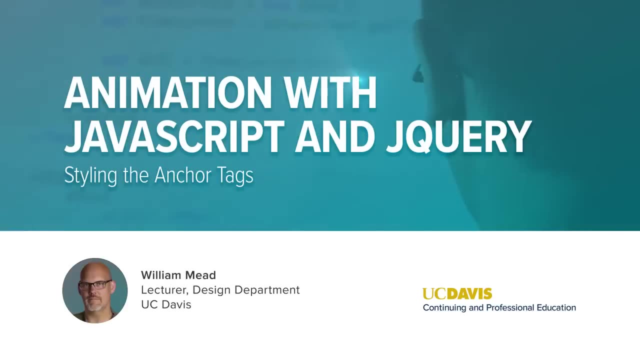 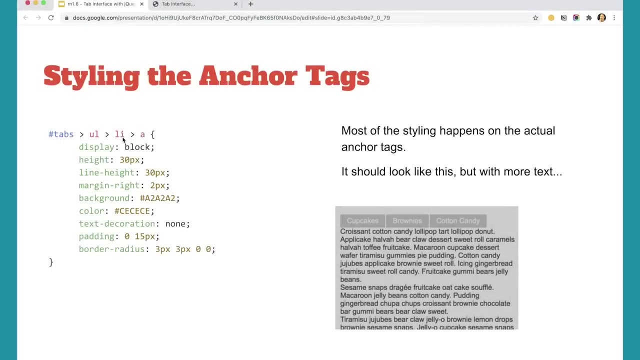 we'll continue with the styling in the next video. the next rule styles the actual anchor tags that are inside the list, items that are inside the unordered list, that are inside the tabs, and again I've got the angle brackets to very specifically get the elements I specifically want. 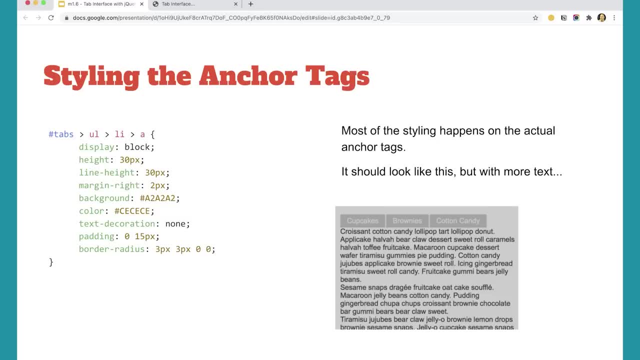 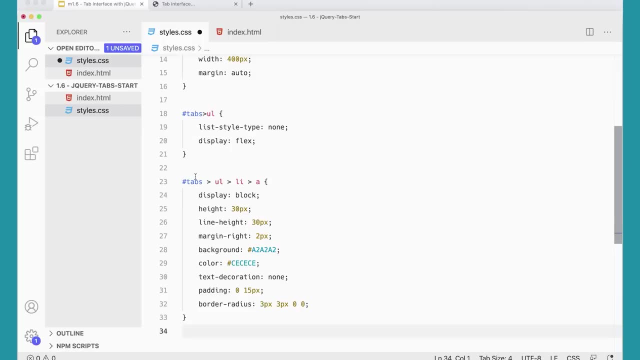 and this is a longer rule, so I'm going to paste it in, but you're going to have to type it. so I'm going to come over here and again, you're going to have to type it. but first thing, I want the anchor tags to display as block elements. 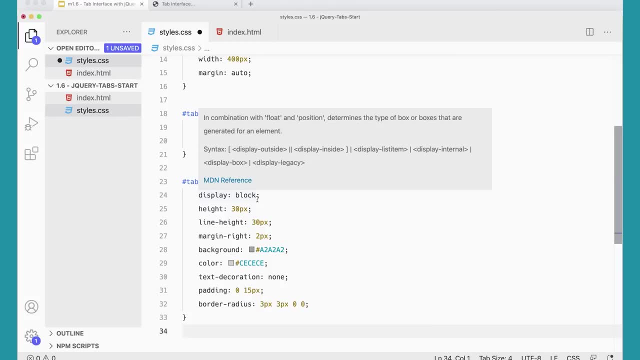 not inline elements. remember, anchor tags by default are inline elements and I want them to display as block. and what that does is it makes the entire area of the tab clickable, not just the text. plus, it makes padding and margin a little bit easier to work with. on block elements: 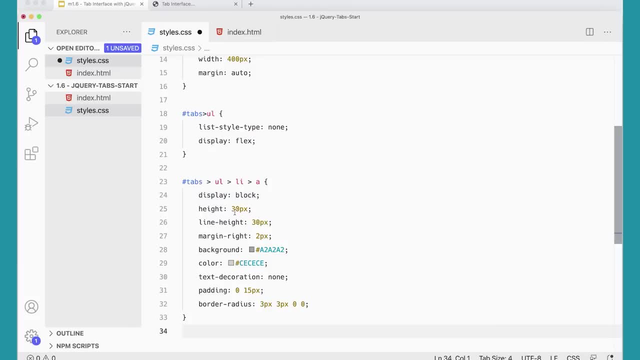 and that will affect inline elements quite the same way. I'm setting the height to 30 pixels and the line height to 30 pixels, and that puts the text in the vertical center as long as it doesn't wrap around. margin on the right: 2 pixels. 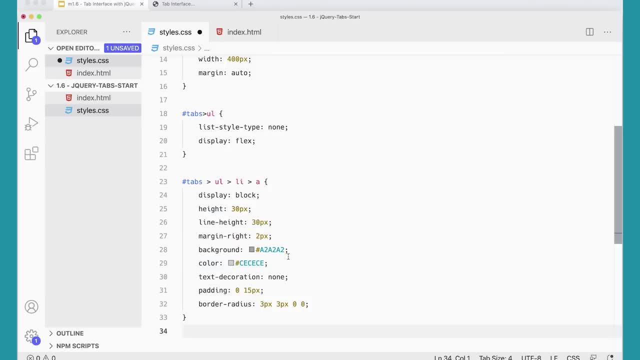 to create a little bit of a gap, and then I'm just setting a background color, the color of the actual font color, and then the text decoration. I'm getting rid of the underlining, putting some padding on the left and right. so 0,, 15 pixels. 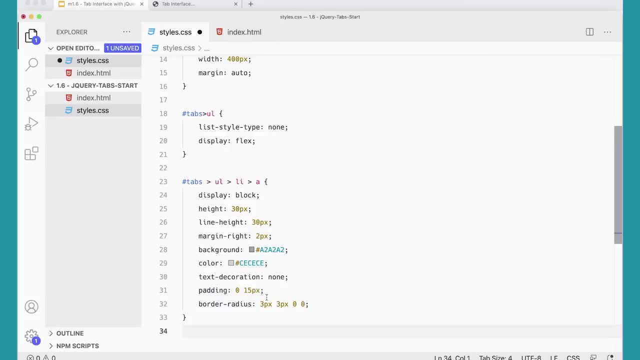 that would be 0 on the top and bottom and 15 pixels on the left and right, and then I'm doing some border radius where I'm putting the border. I'm giving a little 3 pixel radius on the top left and top right of each tab. 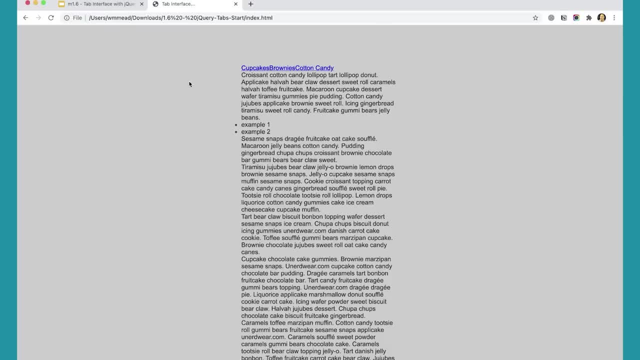 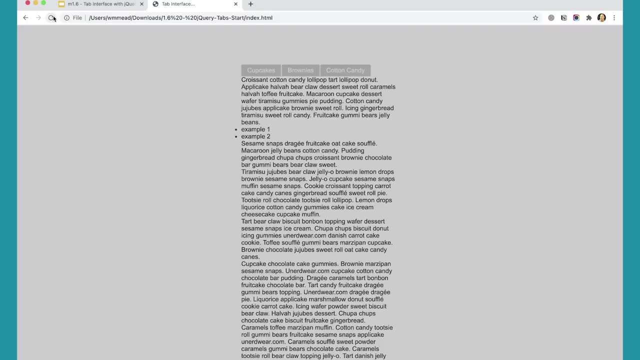 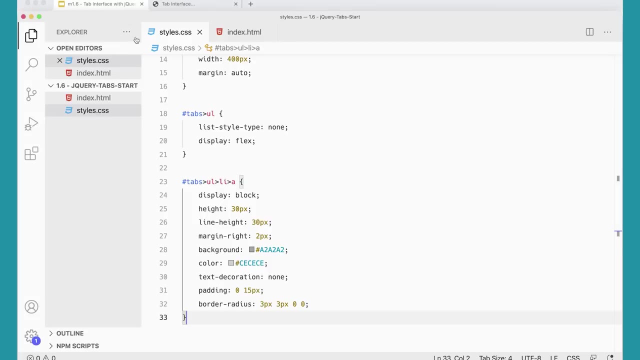 so with that in place, you'll see over here. if you save that, you'll see that the tabs are starting to display the way we want them to display and they're looking like tabs. that's coming along really nicely. we have a few more rules that we need to add here. 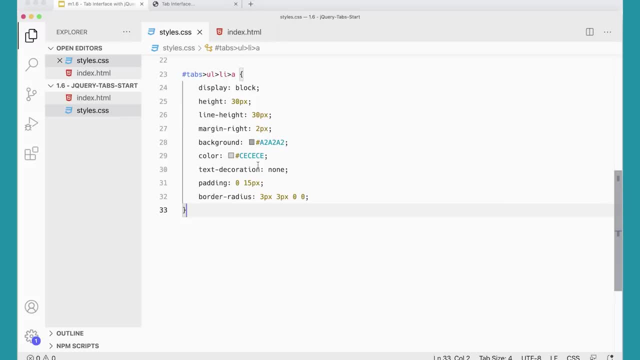 to make our interface look the way we want it to look. so I'm going to add these two rules here. you're going to have to type them in, but this is again going to target the divs that are specifically these divs, the divs that are labeled. 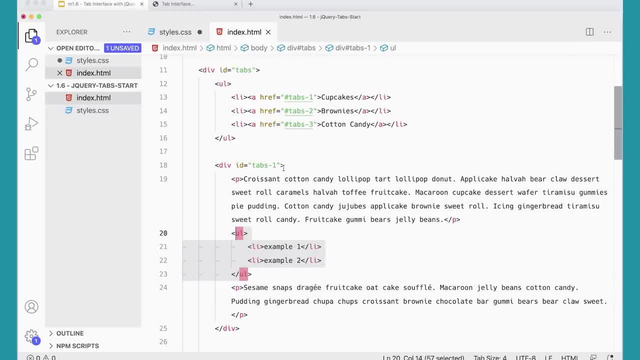 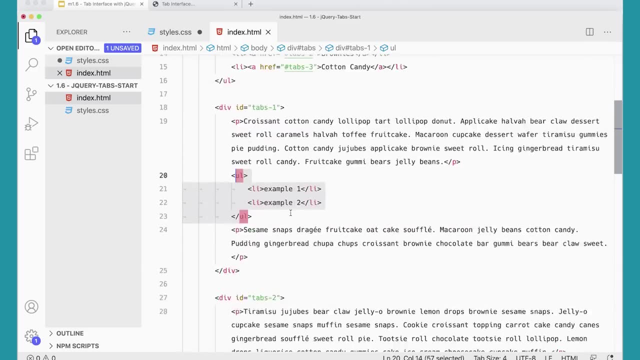 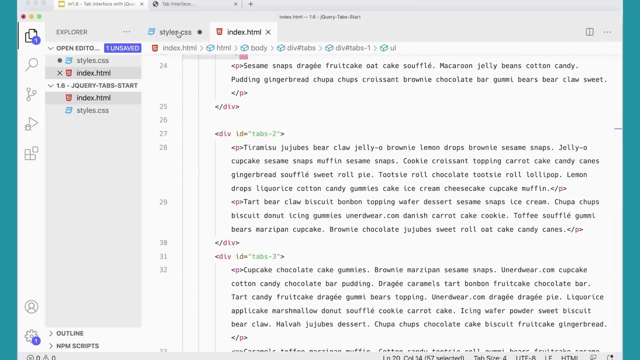 tab 1, tab 2, because again I could add a div in here and I don't want that to be affected. but I want just these divs here, the ones that are tab 1, tab 2 and tab 3, to be affected by this rule. 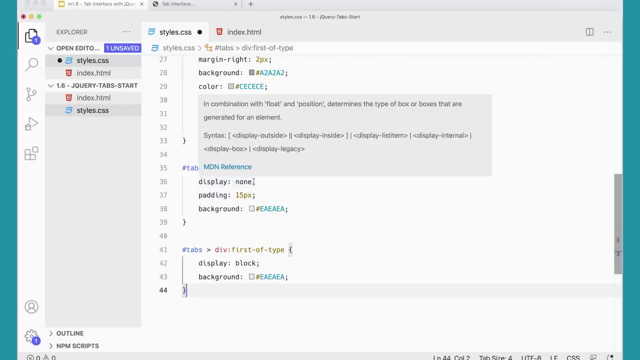 and basically what I'm doing here is I'm setting them so they don't display initially at all, so that hides them all entirely, and then I'm just giving them a little bit of padding and setting the background color, but then the first one, I want the first one- to display as block. 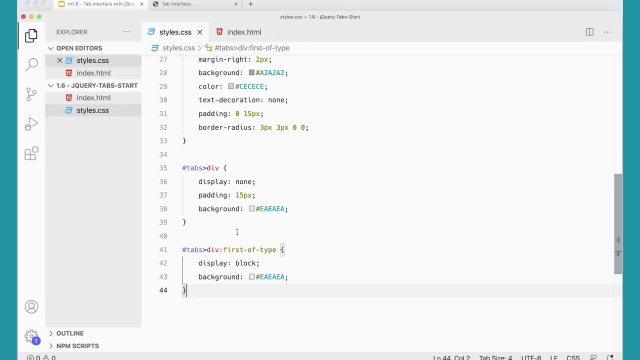 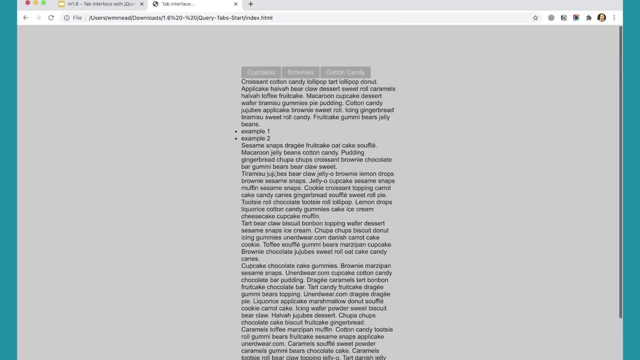 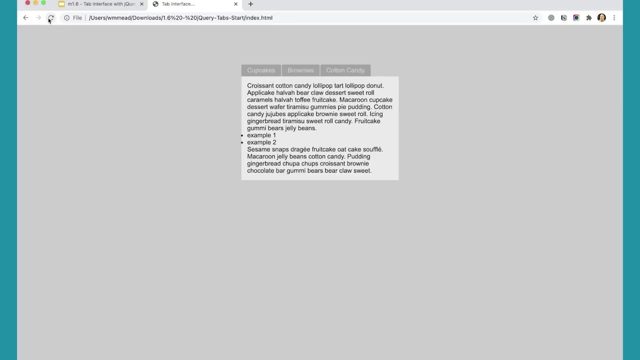 and set its background color. so what that will do you'll see when we come over. here is currently all of these. all of our tabs are showing and really I just want the first one to show. so when I refresh this you'll see the first tab is showing, but the other tabs 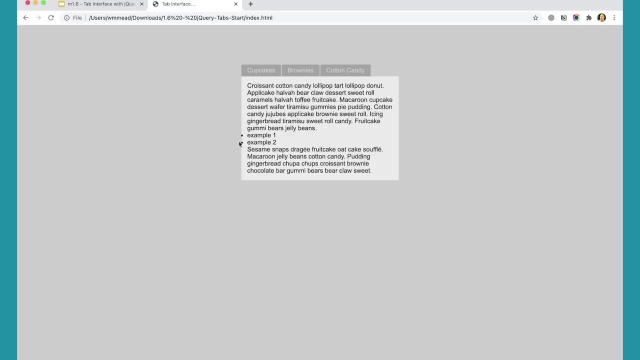 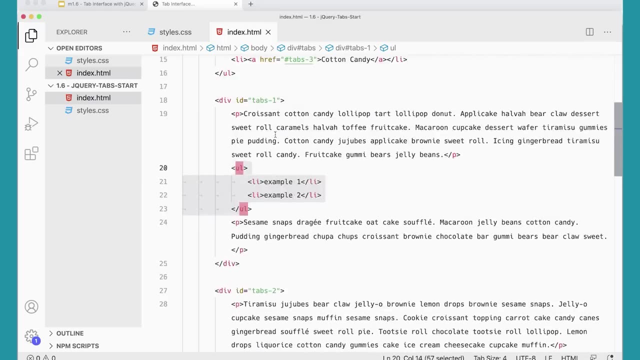 are not, and I'm not going to have styling for this list- I'm going to go ahead and take them out, just because I don't need that stuff in there. I was just to demonstrate that those won't get targeted by the other rule, so I'm going to take that stuff out for now. 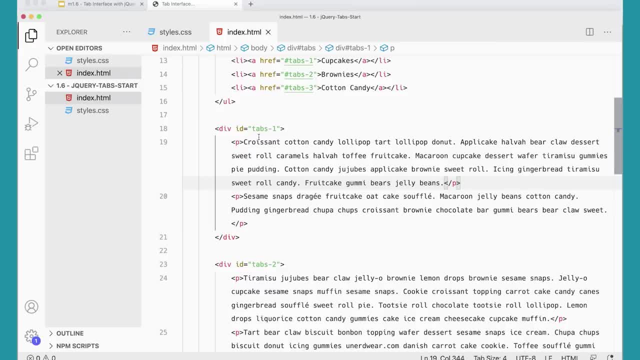 so that's great. and then I've got a couple other really minor rules for styling that will just kind of fix up the way we want our tabs to look and everything to look for this project. switch back to the styles and add two more rules that you'll have to add in here. 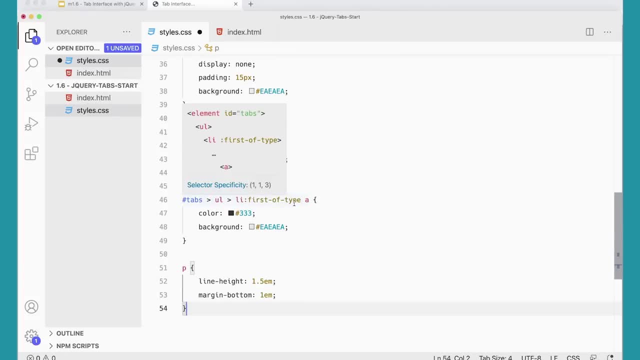 the first one is styling the anchor tags again. this is getting our first tab up at the top of the page and I'm just changing its color and changing its background so it matches our interface. and then I'm just giving a little bit of styling to the paragraphs to make them look a little bit. 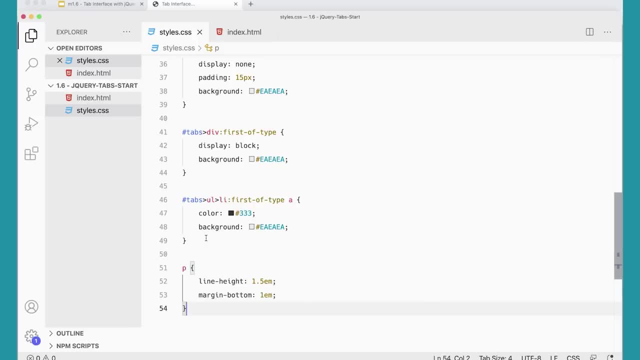 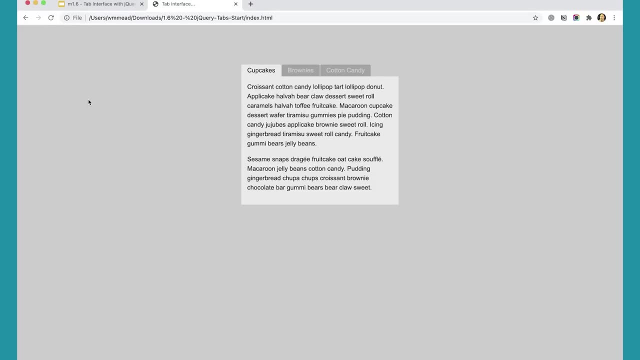 better. so this one isn't super critical, but it's kind of nice to add in there to make our paragraphs look a little bit better here. so now we have the actual interface. it doesn't function, but this is the interface that we want for our tabs and the reason why I showed you the styling. 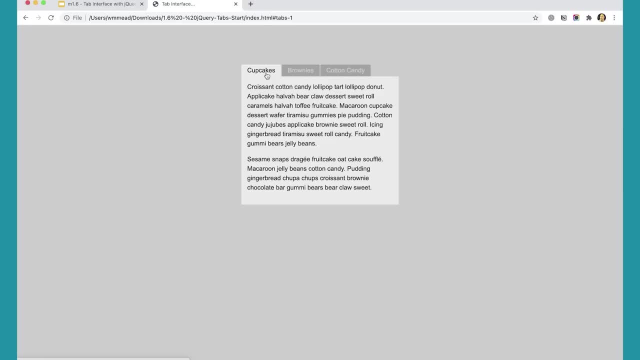 is again because JavaScript is very much tied to the browser and tied to adjusting the styling. it's important to understand how the styling works and that when you're making an interface like this, you want to get the styling for the widget or the element or the interface. 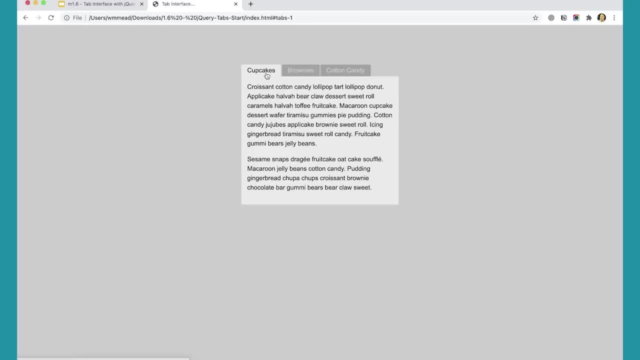 element to work properly before you start working on the JavaScript. so here's the example we have. we have three divs, but two of them are set to display none and one of them is set to display blah. we have an unordered list and they're all styled here. 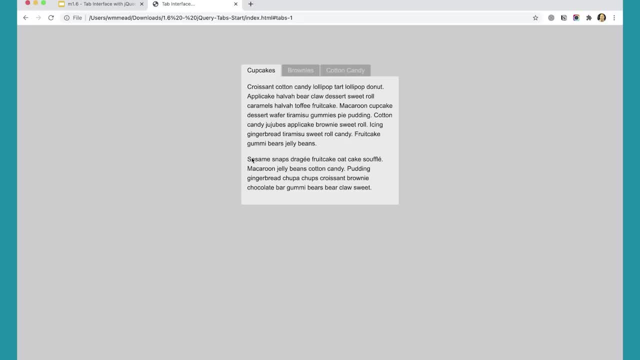 but the first one has a background color kind of matches this thing, so it really starts to look like a tab and we want to get that styling in place. the next step will be to add the jQuery to make the thing actually work, and we'll start working on that. 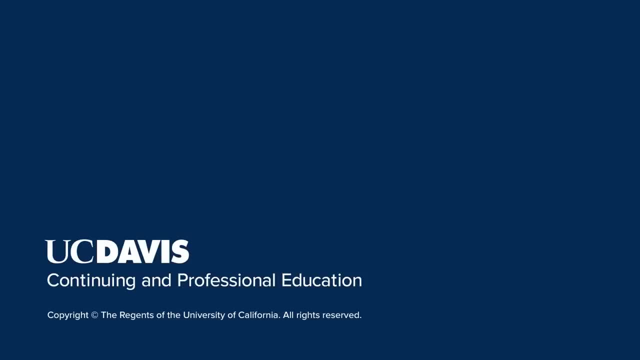 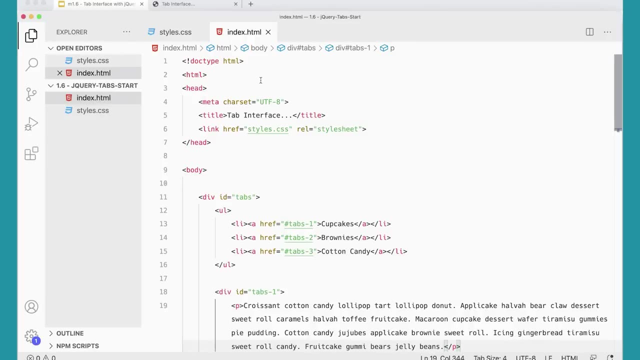 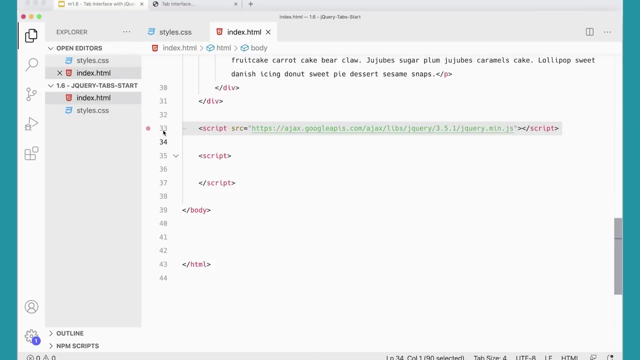 in the next video. okay, now we're ready to start with writing our script to make our actual interface function, our tabbed interface function, and you can see down here at the bottom of this file, I've added the link to the jQuery library. one thing that's kind of. 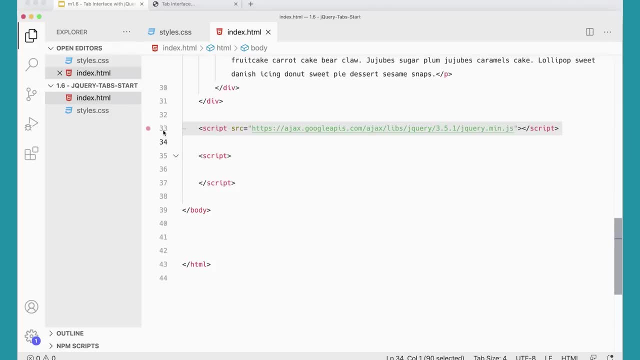 interesting is I was reading online yesterday that they had just released jQuery 3.6, so I'm still using 3.5.1 here and at the time that I'm making this video, if you go to the Google CDN for jQuery, they've not. 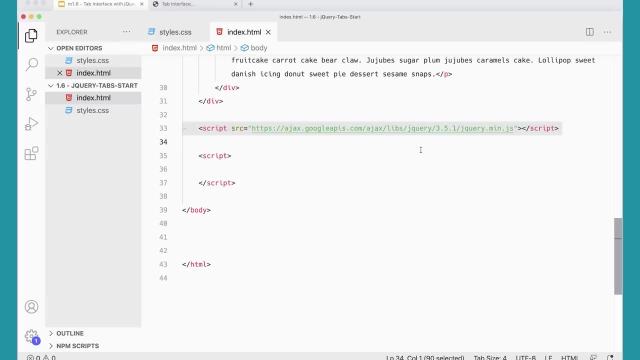 updated it there yet, but eventually it will get updated to 3.6 and everybody's going to have to test out their scripts before switching over. but I don't think it's a very major update, so we'll work fine with this one. that'll work out just fine. 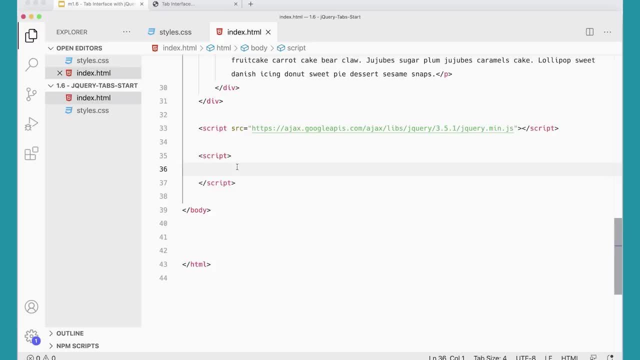 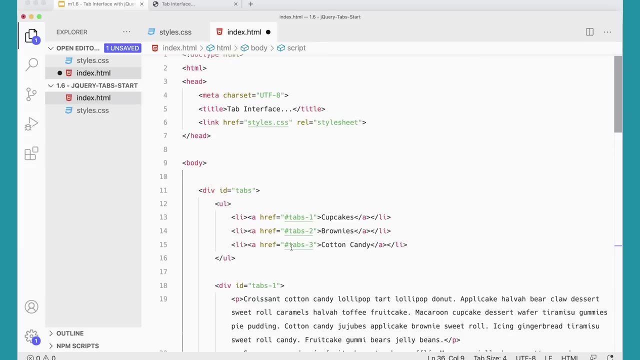 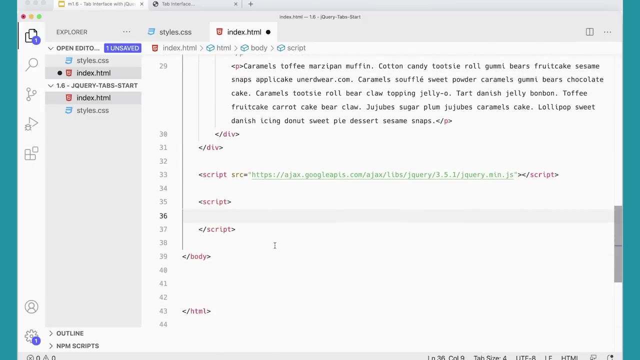 alright. so the first thing we want to do here is add some jQuery to get our to gather all of our anchor tags in here and make it and add it, so when you click on these, something happens. so again, we're going to use our jQuery object, as always. 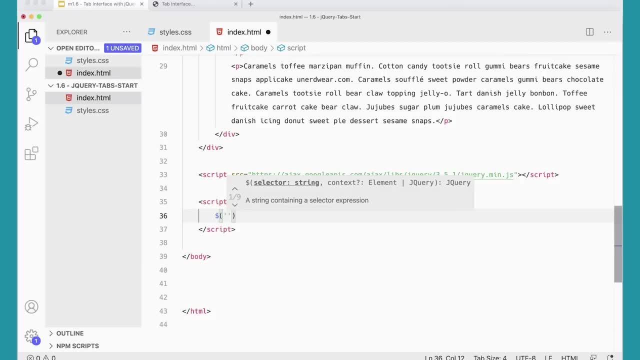 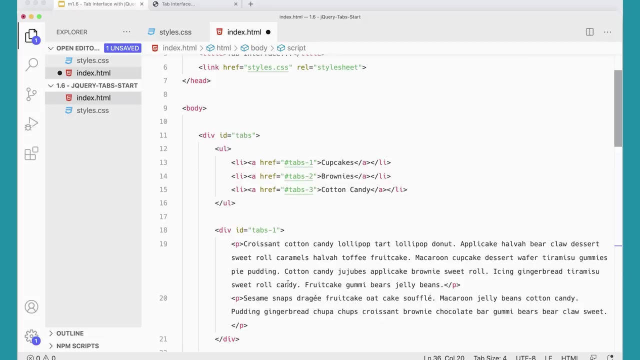 and in here again, I want to very specifically target the ul angle bracket, ally angle bracket a. or, even better, I want um pound tabs angle bracket, ul ally a. because I want to very specifically target these anchor tags, not any other anchor tags anywhere else on the page. so that's why. 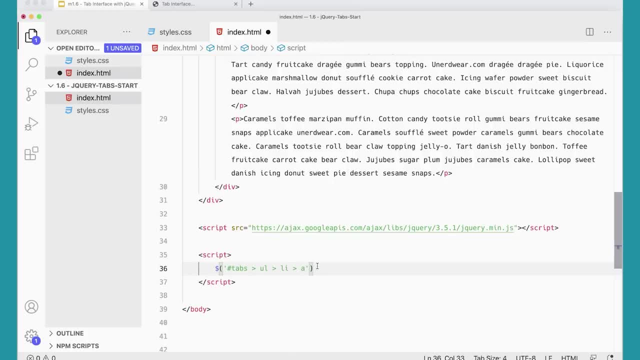 I'm using the angle brackets in there, so I want to target those. and then I want to add a click handler: click so that when click something happens, and of course I come in here and, as we've done before, add a function that runs, an anonymous function that runs. 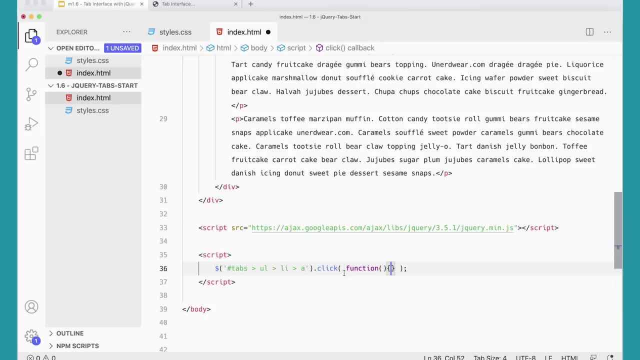 when you click these links, so this anonymous function will run and, as always, I'm typing from the outside in so that you can really make sure that you don't lose any curly braces or semicolons or anything like that, and then I can click inside the curly. 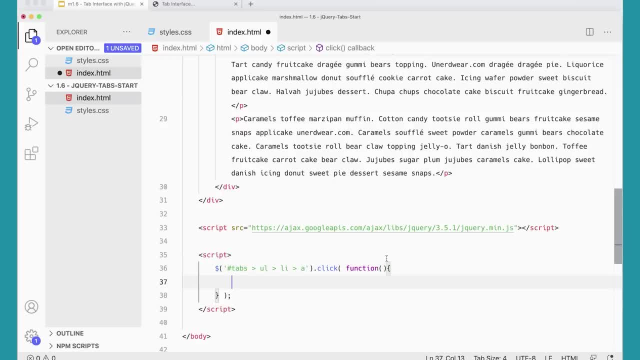 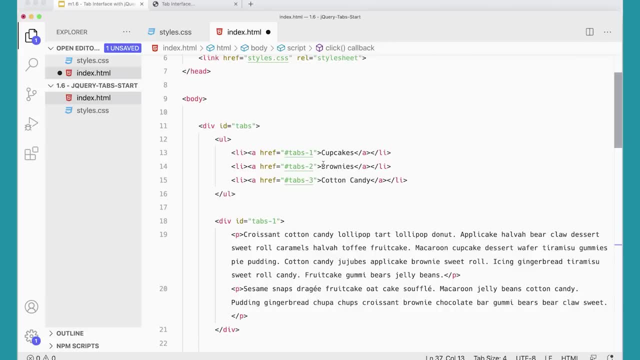 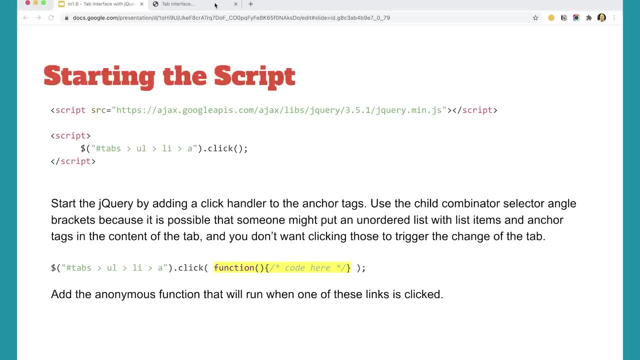 braces, and in here what I want to do first is I want to, I want to get all of these anchor tags here and make it so that the background color, the color and the background color of these are all set to the default background here, this default color. and then I want to take 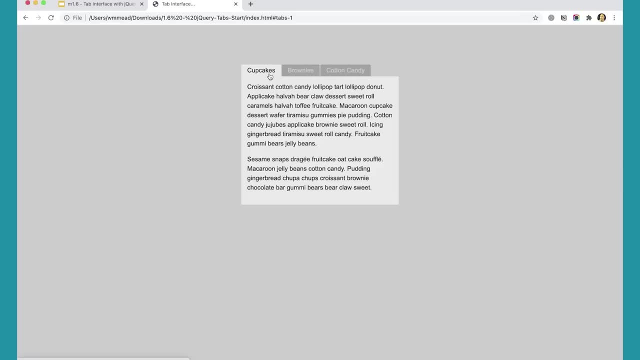 the one that I clicked on and change its background color to this color and its and the color of the font to this color. so I'm going to change two things in these, in this click handler. I'm going to change this background color and this and then that that one there. 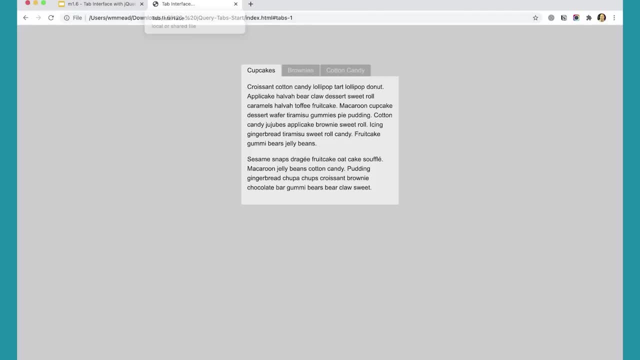 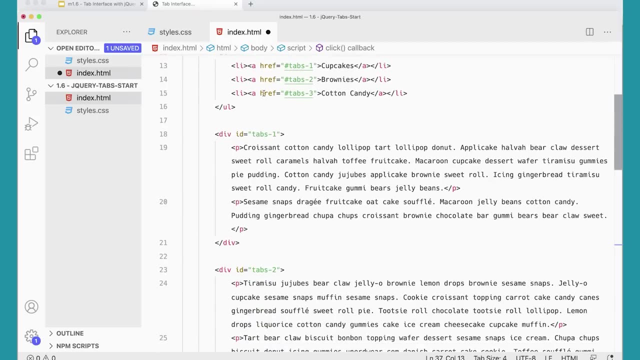 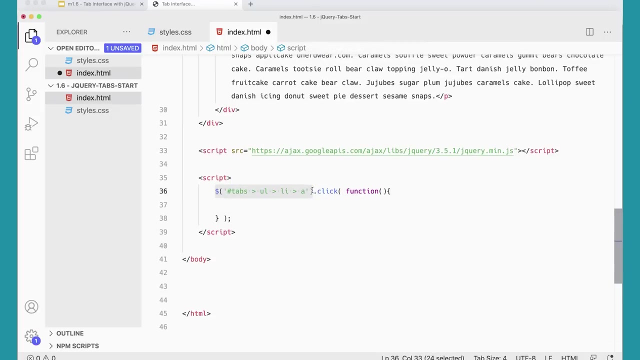 so, again, what I want to do here is: I want to get, I want to get these same anchor tags, so down here, I'm actually going to copy this and I'm going to effect these elements that I'm already getting here. I'm going to get those. 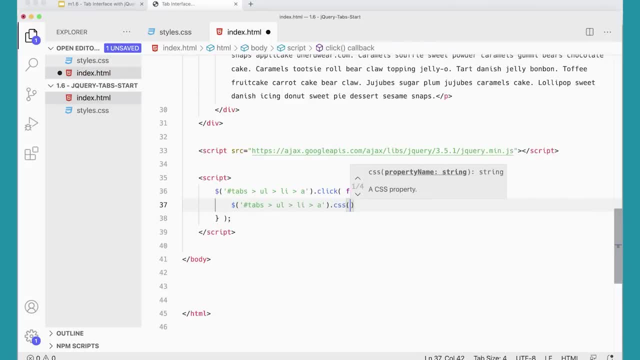 and I'm going to do dot css and before, when we did css and we did, we did something like this color comma. you know you could do green or you could do whatever you want and pass in a two variable, two, two arguments that are the that are: 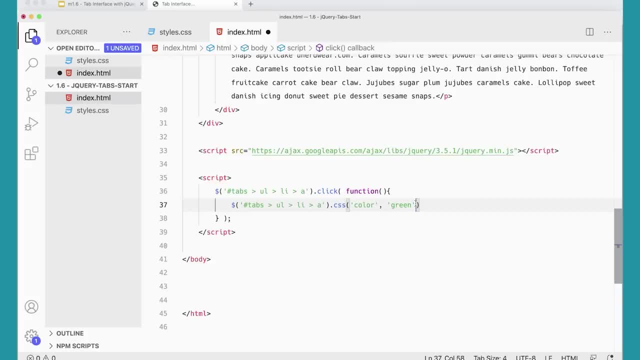 setting the color to green, like this, but you can also use this method with an object if you're going to set multiple things, and that's what we're going to do here. we're actually going to set multiple things, so I'm going to put an object in here. 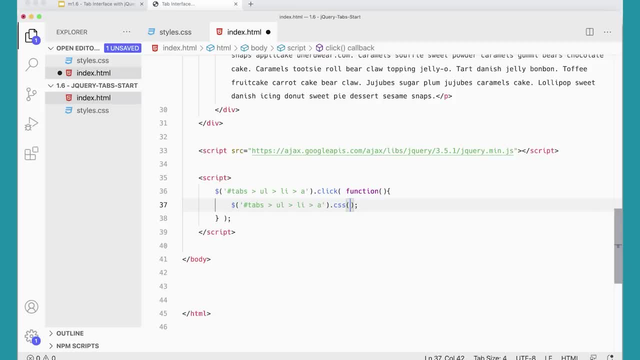 we've talked about objects briefly. we'll get into objects later on in our lessons. we'll get more deeply into objects. but an object starts with curly braces and we pass in key value pairs that will work with this object, and the css method in jQuery allows you to do this. 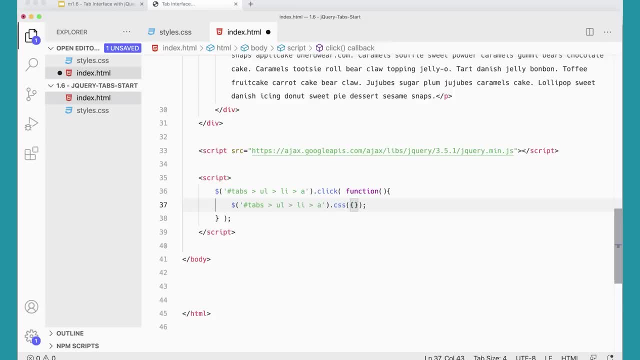 if you can set multiple things- and we do want to set multiple things because we want to set the background and the color, and we're going to set background and that doesn't go in quotes because it's the property and we're going to set it to. 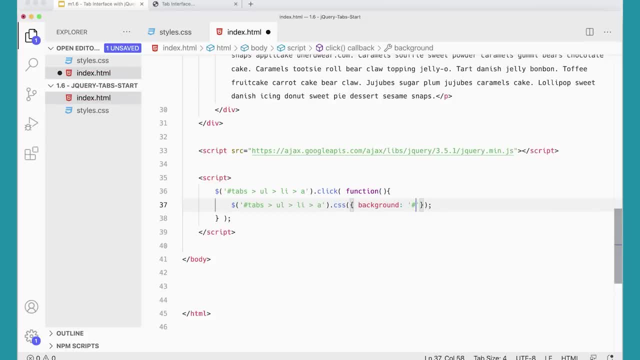 this one does go in quotes: pound a2, a2 and then a comma and we're going to set color colon and it's property is going to be pound cece. so that's going to set these colors. and again, where am I getting that? that's coming straight from the styling over here. 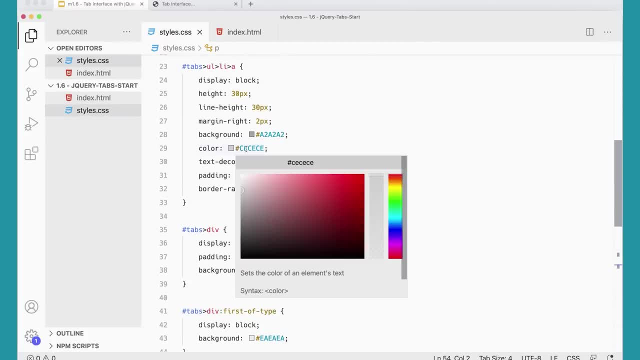 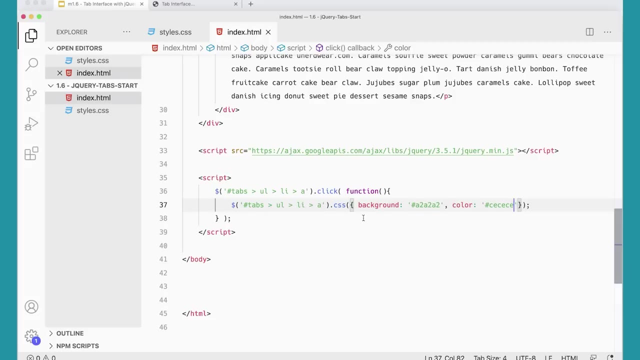 so these tabs, the color of the text is this lighter gray and then the background is this darker gray. so that's where that's coming from and that's where I want to set these to, so they immediately all get set, all of them get set to the color. 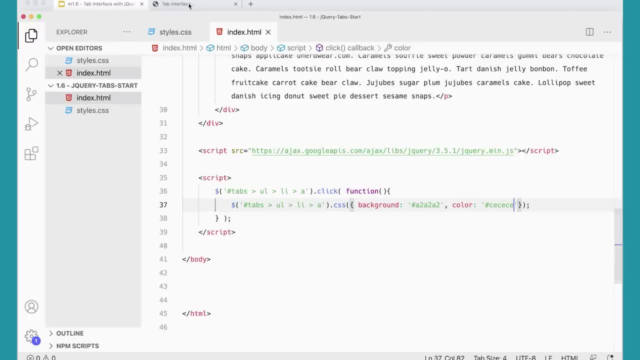 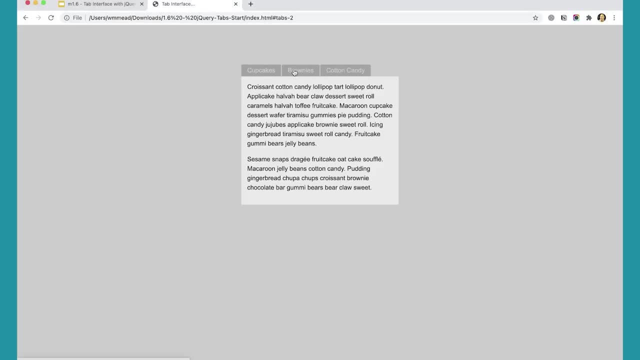 of the background. and if I come over here and test this, as soon as I click on one of these, you'll see they'll all turn to that dark color. then I want to take the one that I clicked on, this one- and set it to this color here. 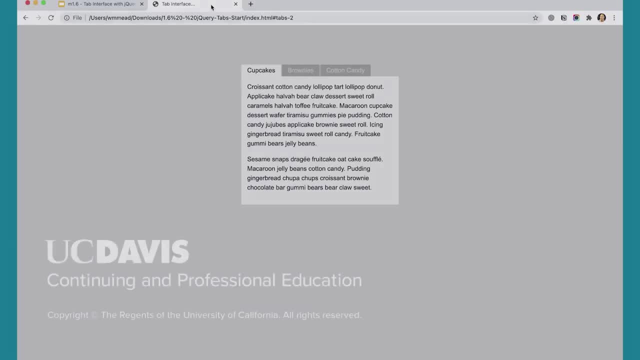 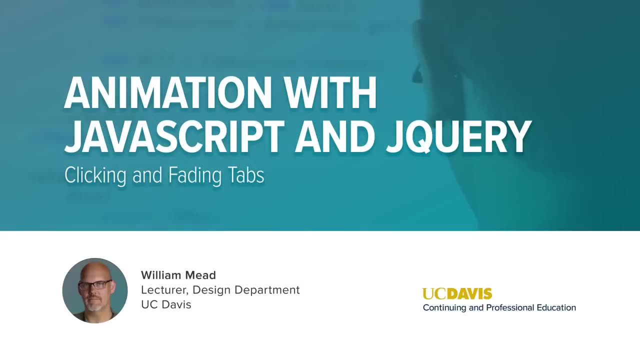 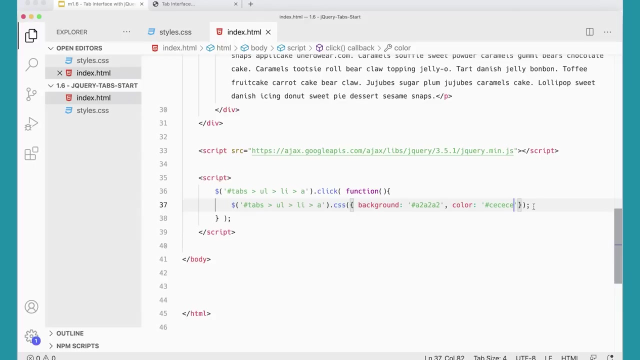 so we'll do that in the next video- all of the backgrounds to the default color. now we need to turn the background and the color of the font for the one that we've clicked on, and again, you can only click on one tab at a time, so which one did you click on? 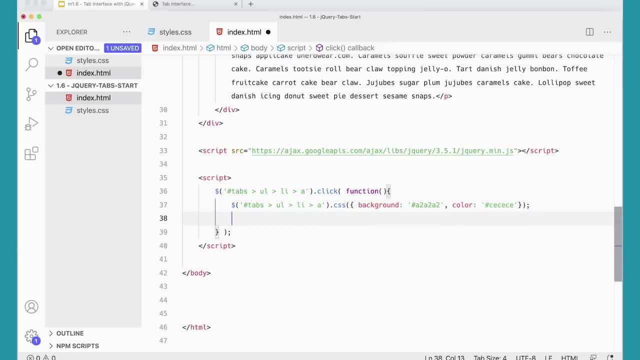 you clicked on this one. so we're going to use the this keyword, dollar sign, this, and then we're basically going to do a CSS command like this here, so I'm going to copy that and paste it here and then, but the colors are going to be different. 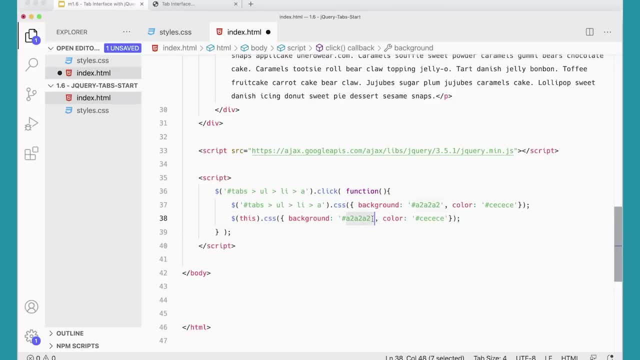 the background is going to be EAEAEA, I think, and then the color is going to be 333, like that, and that should work. let's save that. and, um, when I come over to my tabbed interface here and click refresh now, when I click on brownies, 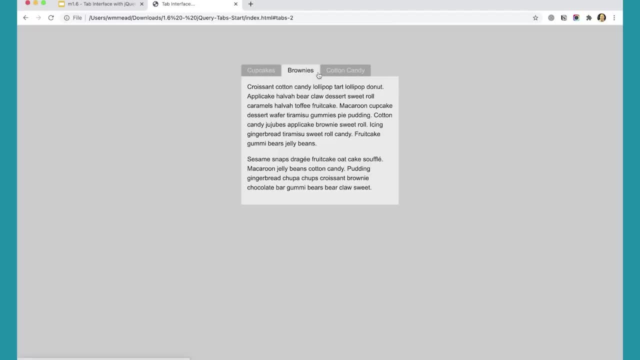 you can see they're all turning to black, they're all turning to dark gray, and then this one, the one I clicked on, is turning white gray, so it makes it look like this tab is active. now we've activated the tab, but we haven't actually changed the tab content. 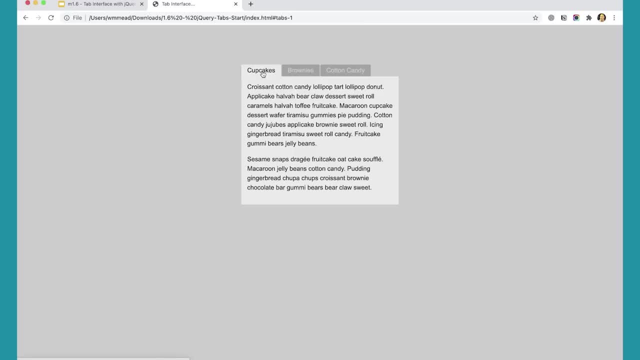 so that's what we're going to do. next is change the tab content so that, when we click on this, the correct tab content shows up here. so how are we going to do that? well, when we click on one of these, there's an href attribute. 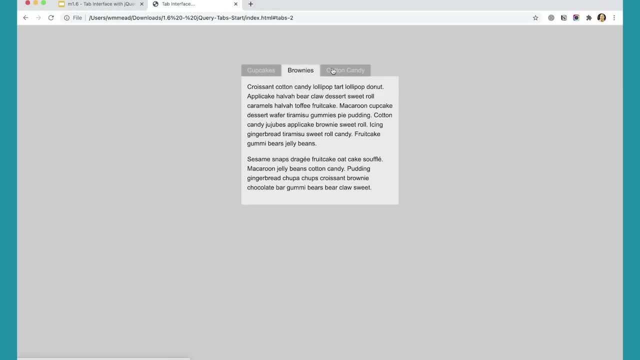 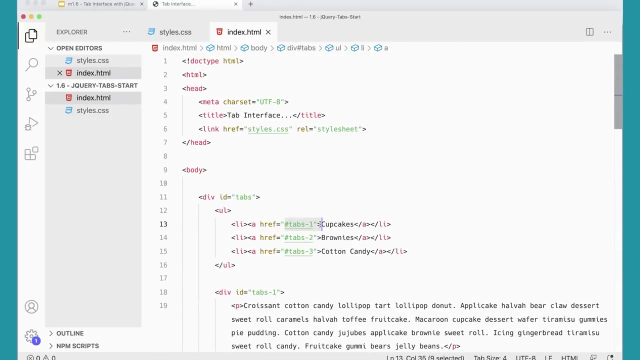 associated with this link and we know that the href attribute that's associated with these links is also associated with the content below, because that's how we had our markup set up over here, remember up here. we set these hrefs here to link to these IDs down here. 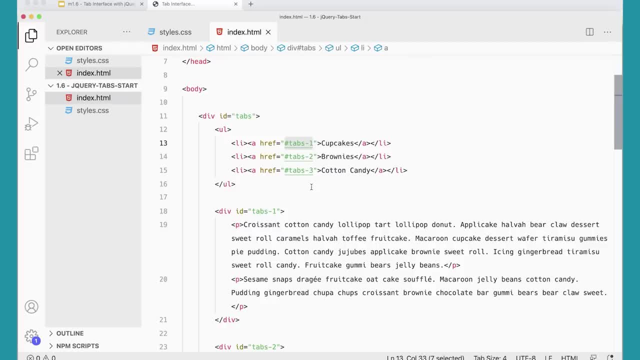 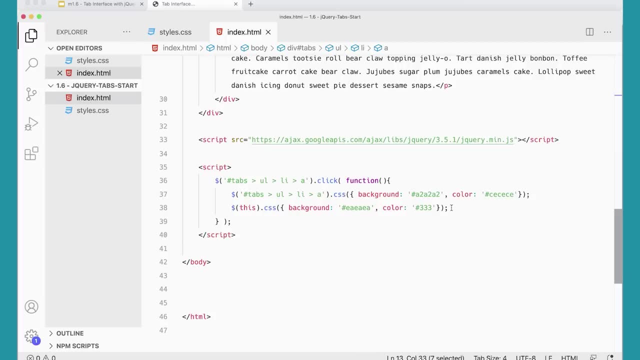 so really, what I need to do is find out what href I clicked on when I clicked on one of these, so we can do that very easily down here again using this keyword, I'm going to make a variable var thisTab and I'm going to assign it. 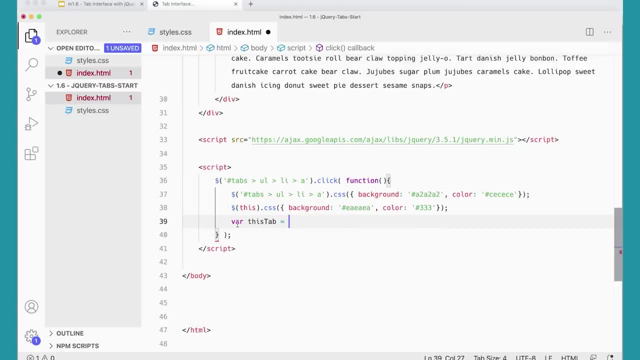 a value. it could be var or it could be const. I'll just use const for now. I'm going to use this keyword I'm going to use in our jQuery object and I'm going to use attr, which is the attribute method in jQuery that allows me to get: 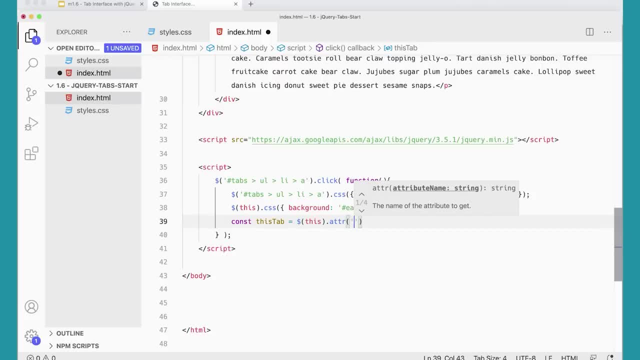 a particular attribute on an element. what attribute do I want? I want the href. and just to see what's going on with this, if I do alert this tab and see what I get when I do this, you come back here and refresh the page if I click on brownies. 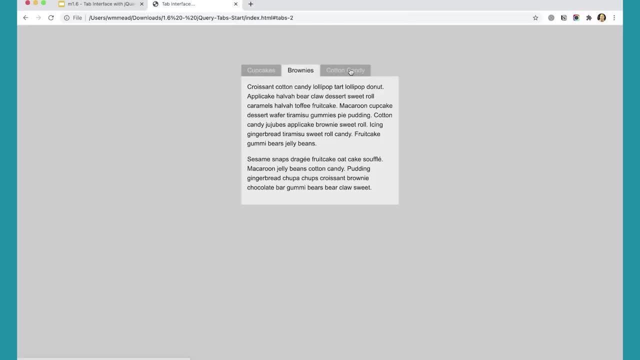 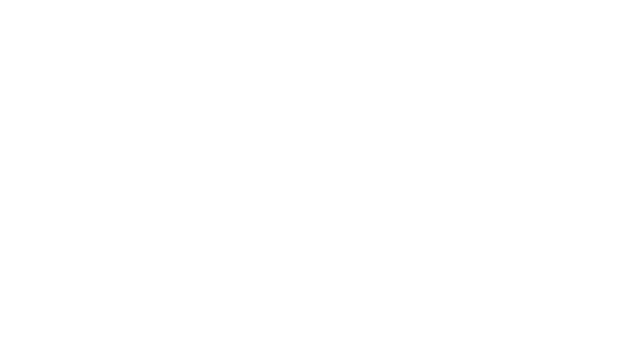 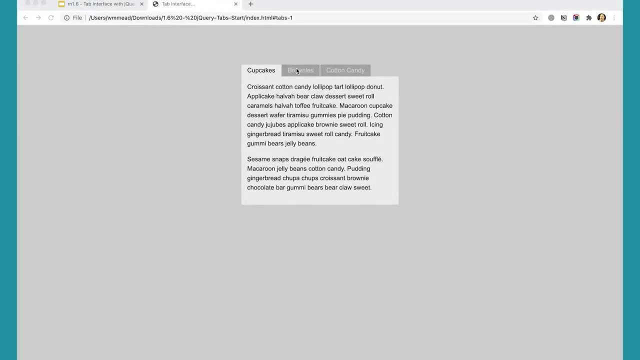 I'm getting pound tabs too. if I click on cotton candy, I'm getting pound tabs three. if I click on cupcakes, I'm getting pound tabs one. so that's getting me the correct tab, which is exactly what I want. now that we have that working and we're able to, 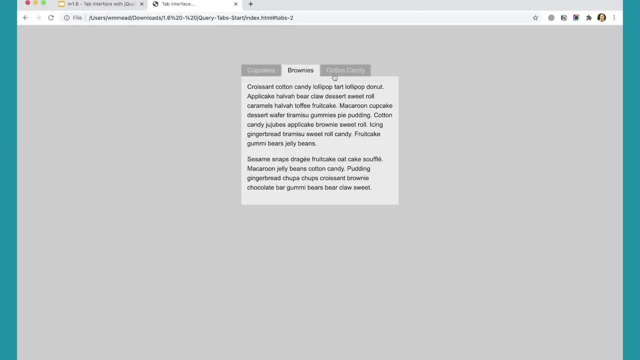 click on these and swap out the correct information there. what do we want to do? how do we want to actually handle this content here? and what I want to do is actually want to fade out this content that's showing for the tab that's selected and then, when that's done, fading out. 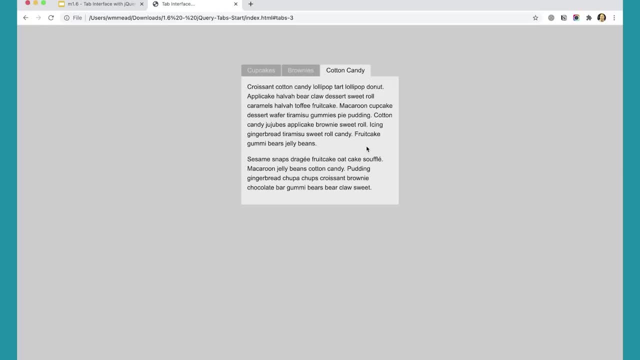 fade in the new content and that fade, that animation, is going to be handled by the jQuery effects library and it's very simple. it's going to happen very quickly. it's going to happen in 200 milliseconds, so a split second. but that fade is important to the interface. 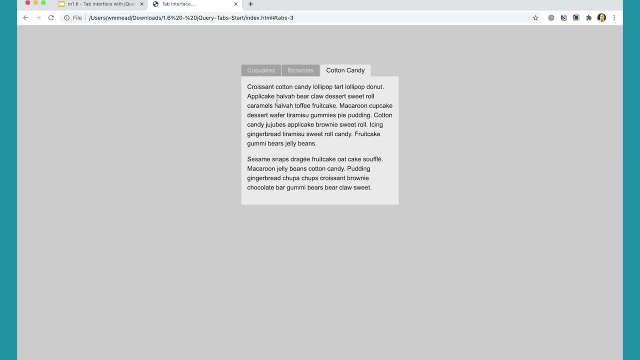 that the information is actually changing, because the information in these tabs doesn't look all that different in these content areas. we want to do that animation so that we can actually show the user that when they click the tabs it is actually changing and getting some different information. 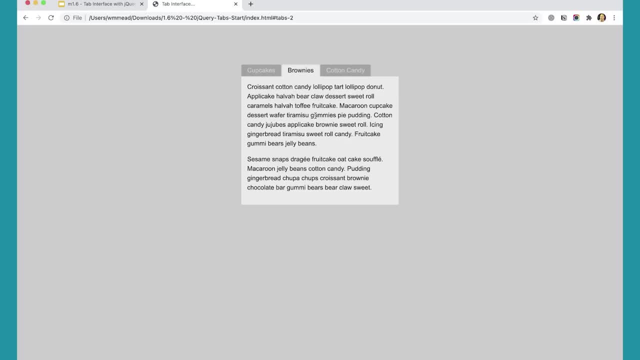 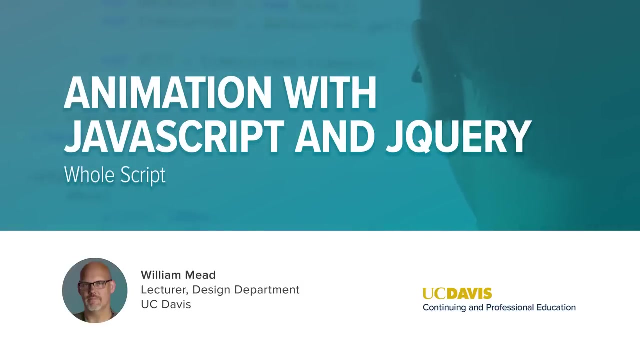 in there. so that's what we'll do in the next video, and we'll finish this thing up and you'll see how the interface looks when we're done. alright, so now we need to fade out the current tab that is showing and we can get rid of this alert. 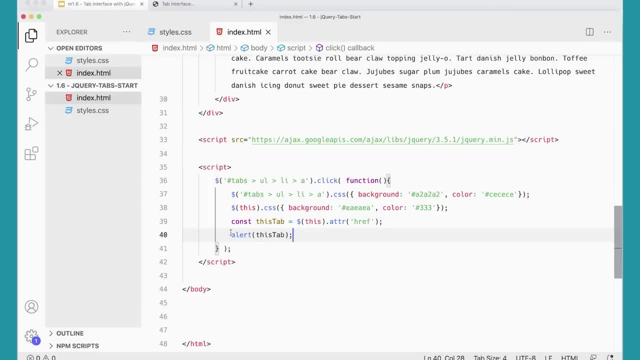 you can either just comment it out if you don't want it there, or you can delete it, but we don't need that anymore. but what I need to do is I need to get the particular tab that's currently showing, and we can do that using jQuery. 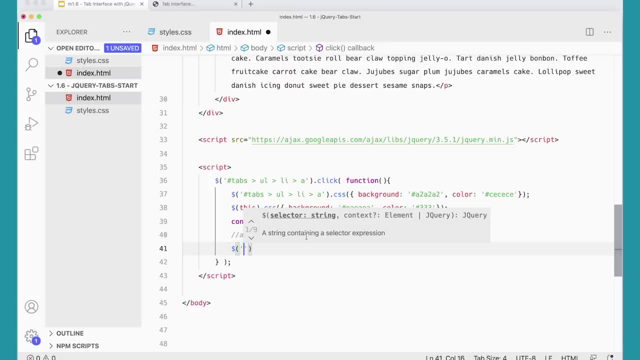 and remember, in jQuery there's always so many different tabs and other ways of getting to elements on the page and in this case, I think the most effective way is to use tabs. angle, bracket, div, colon visible. we've talked about this filter before briefly, and it will. 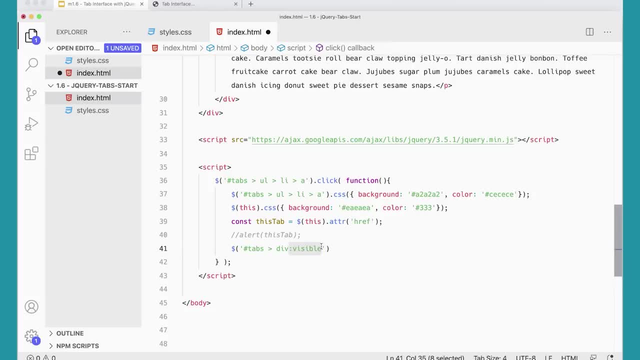 give us. whichever one is currently set to display block. so that's the current one that we need to set and we're just going to set it to dot fade out over 200 milliseconds and that will fade out the current one that's showing. so the other ones are all set to display none. 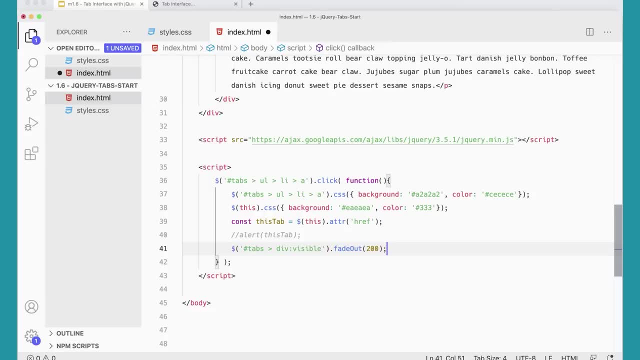 so that will fade that one out. so now they're all set to display none. so what do we need to do once we finished fading this one out? is we need to take the one? once this animation is finished, we need to take the one that we clicked on. 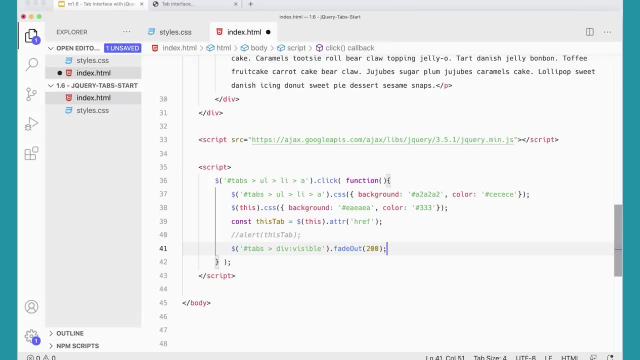 and fade it back in. so that's what we need to do next. so what we need here is a callback function. remember that's how the callback functions work. so once this is done- fading out- we want to add a callback function function with its parentheses and its curly braces in here. 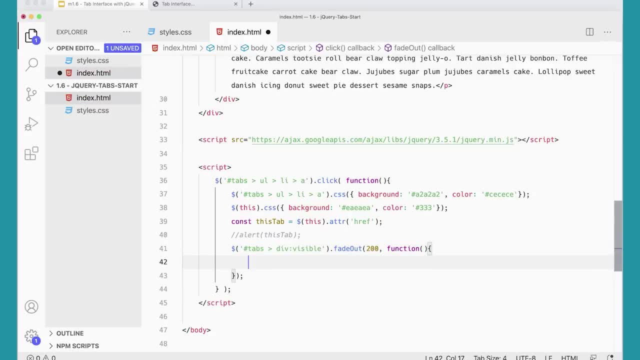 I'm going to click enter to move that down, just to make some space, and then I'm going to say, okay, I want this one, the one that I have currently clicked on, I want this tab to be to- to get faded in. so the way we're going to do that, 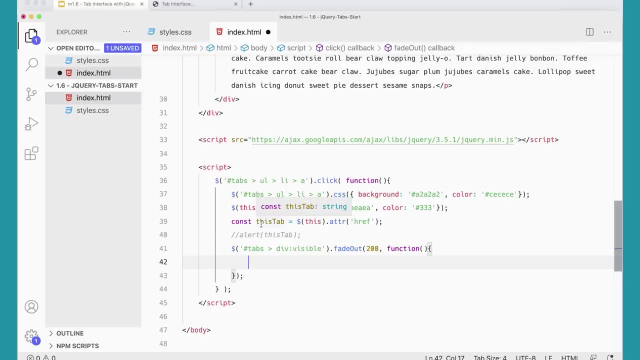 is, we're going to make use of our variable that we've already created here. so we can do. we can use our jQuery object to get this tab and we know that this thing we can hold in it, either, or because that's what we found when we did this alert. 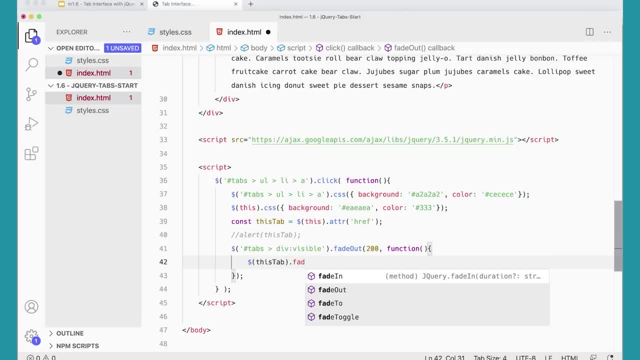 so we can get this one and then we can do dot fade in over 200 seconds, 200 milliseconds, so it will fade that one in great. so now we have a nice, simple little script that allows us to use these elements and use the jQuery effects library. 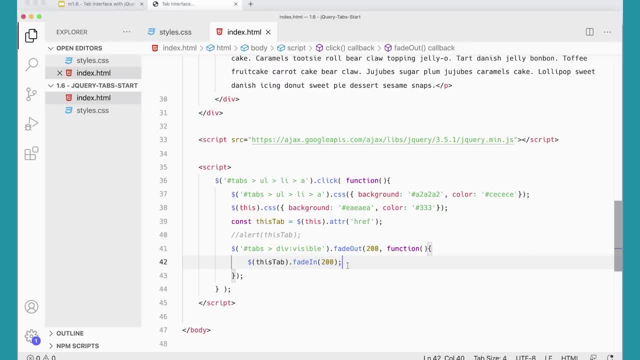 to fade them in and out and you know this isn't particularly heavy duty effects library stuff. it's not going to look terrible on mobile or anything like that. we're just doing something very simple here. this is a really good use of the effects library, so let's see if this actually works. 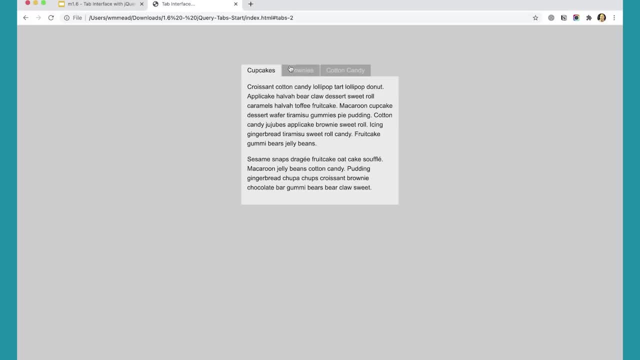 come over here, refresh the page. when I click on brownies, it fades the first one out and that's working perfectly. and because of the animation, it's giving us a sense that the content is actually changing. so it's a really good use of the animation there. 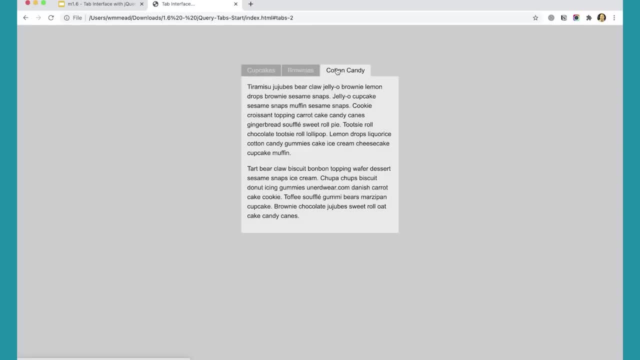 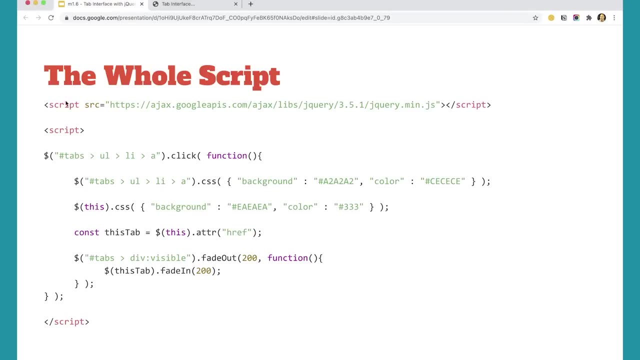 and of the effects library. so that's working great. let's just review the whole script. so here we're loading the jQuery library and then in our script we're getting those anchor tags and adding a click handle. a function runs when they're clicked. we're changing the tabs. 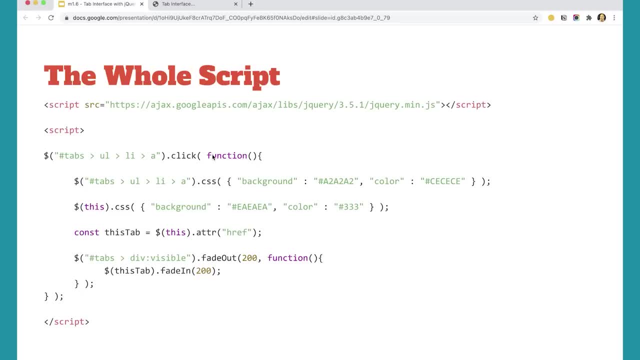 we're changing all of them to be the default background color, the unselected color for both the background and the color of the text, then the one we clicked on, we're changing so that it shows the correct color and text for that one. we figure out. well, which link did we click on? 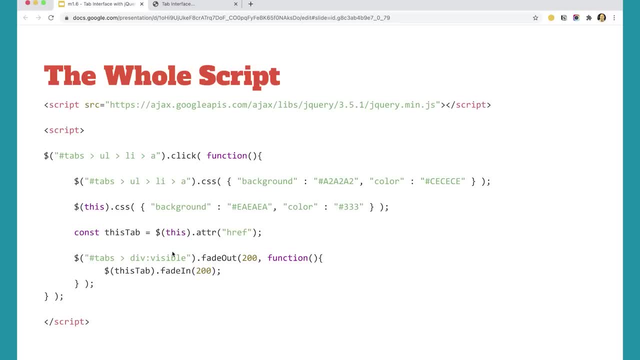 and then we're going to take the corresponding div that goes with that, fade out the one that's currently showing and take the corresponding div and fade it back in and that's the entire script. so it's a nice simple script and does a nice job of making use of. 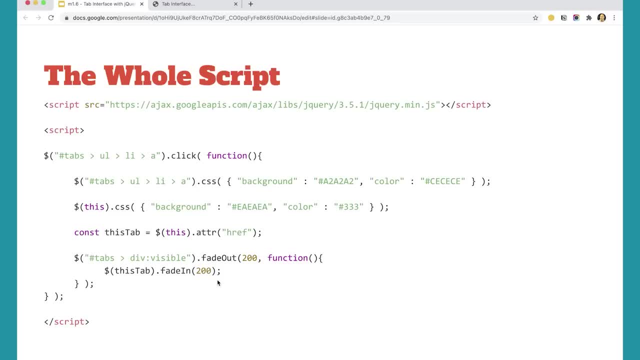 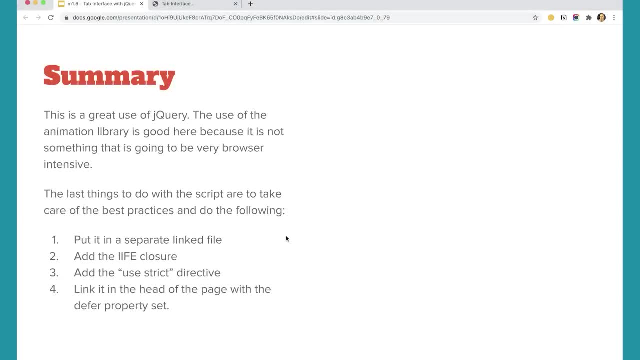 our effects library in jQuery to build something simple and effective that you can use on lots of websites. so again, in summary, this is a great use of jQuery. maybe if this is the only thing you're putting on your web page, that would use jQuery. it's not really worth it. 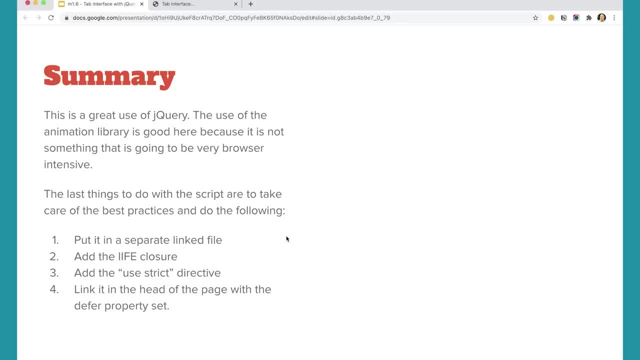 because you're downloading the entire library just to make these little tabs, and we'll see how to do these same tabs in plain JavaScript. but it's working really great and if you are using jQuery for other things on your website, then this would be a really good use for it as well. 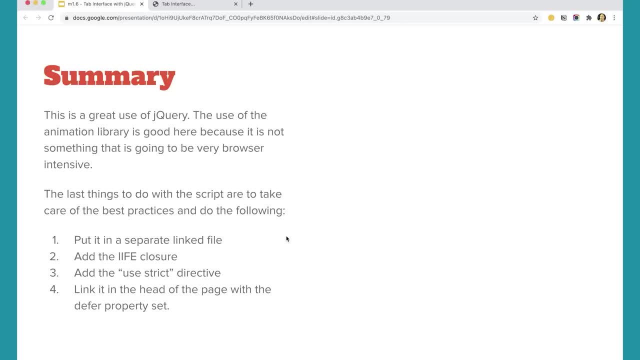 the last thing to do here is just put the script in a separate link file, iife the immediately invoked function expression closure and add the use strict directive and link it in the head of the page with the defer property and do all that stuff. so let's just go do that really quickly. 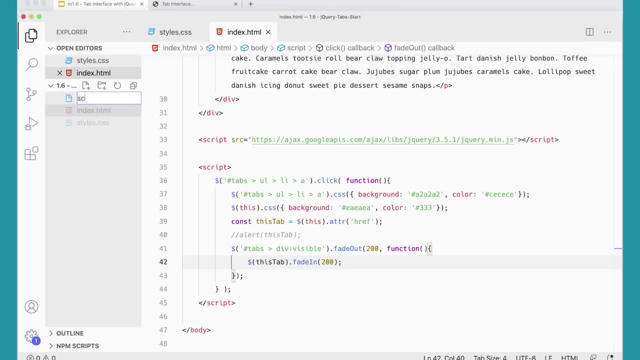 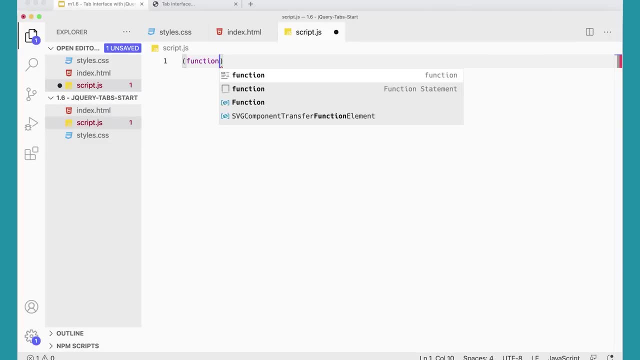 while we're here. so here I can just make a new file called scriptjs, and on that file I can add my function, parentheses, curly braces and an extra set of parentheses at the end to make it run. and then inside the curly braces I'm going to add my 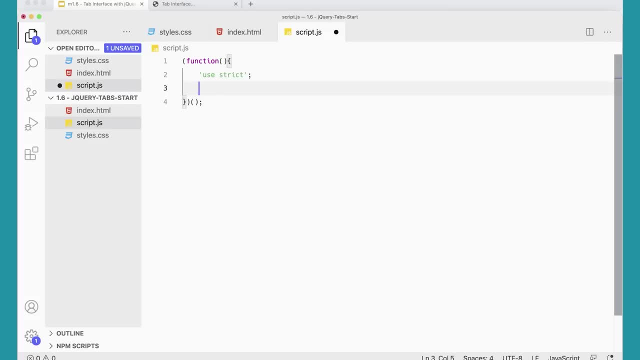 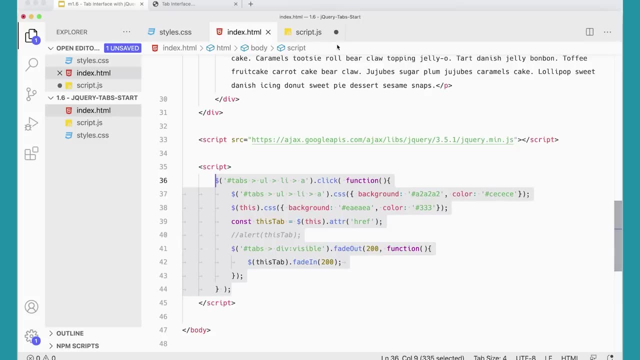 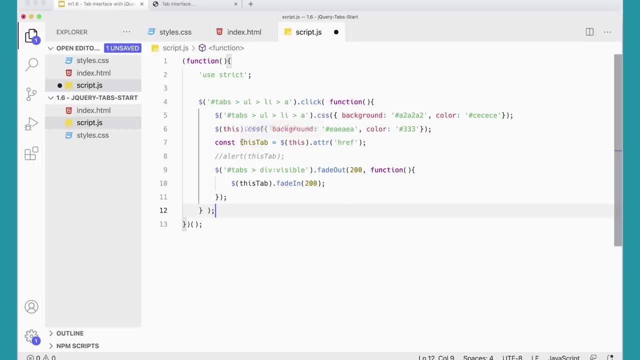 use strict directive semicolon, and then I'm going to come back here and just copy this script from here. I already used const for the one variable that I have, so I don't really have to do anything with that. so that's all fine. that should be all good there. 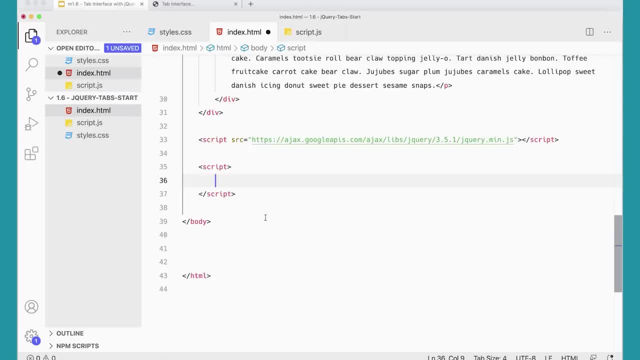 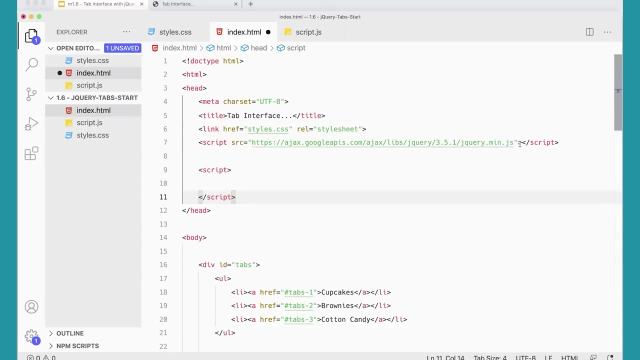 I'm going to just get rid of this stuff. instead, I'm going to move these things up to the top of the page, cut them from here and stick them in the head, but again you have to add the defer attribute here, like that. and then for this script here: 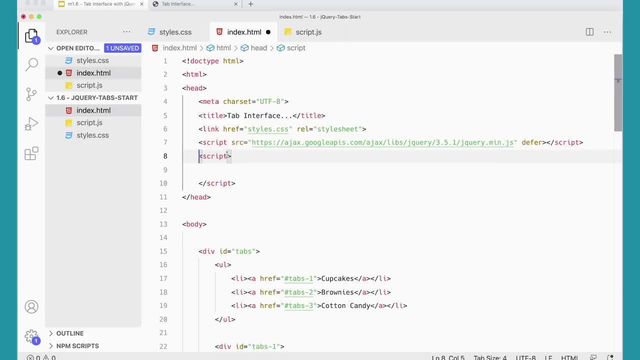 I'm just going to link to my script tag, so I'm going to just src equals, quote script dot js, and then- don't forget, defer, and then this thing down here can go up to there. it was there we go, and that should all work. let's just test it really quickly. 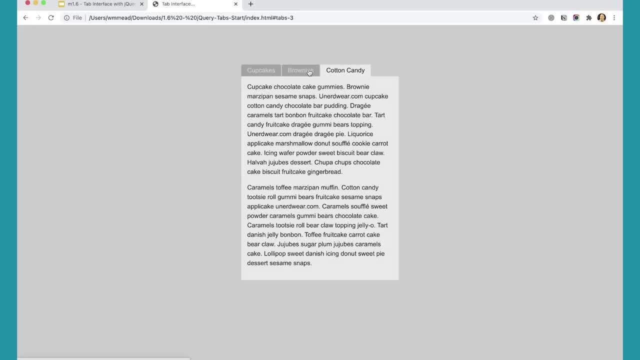 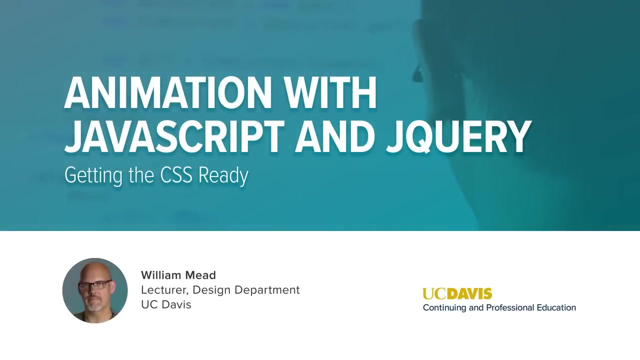 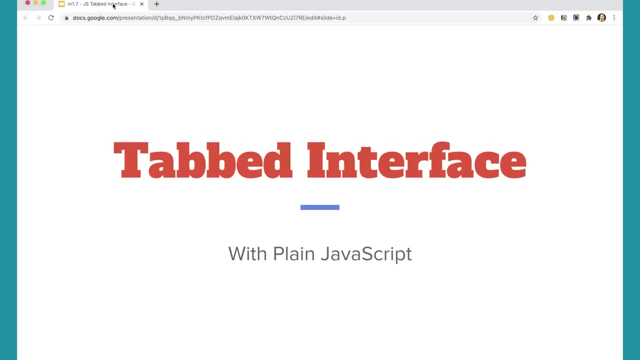 and make sure it works. and it's working great and we've got kind of a nice clean, simple script that we can use using jQuery. now that you've created the tabbed interface using jQuery, we're going to create that exact same tabbed interface using plain JavaScript. 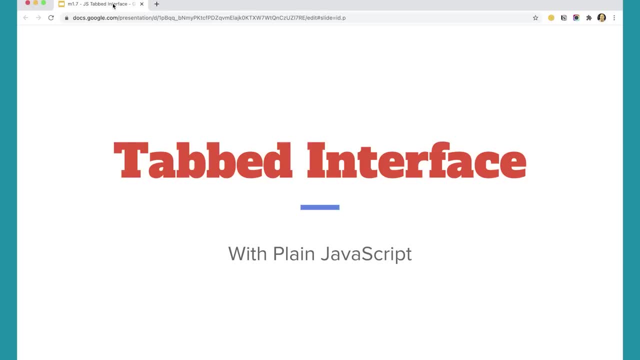 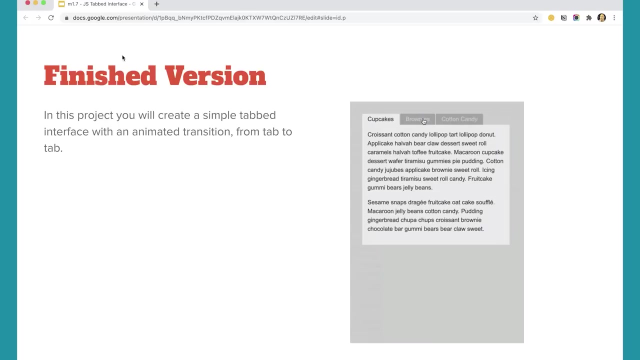 and that way you can compare the syntax between the two and understand the difference between plain vanilla JavaScript and jQuery and making use of the jQuery library. so when we're done, the interface is going to look exactly the same and function exactly the same as it did before using jQuery. 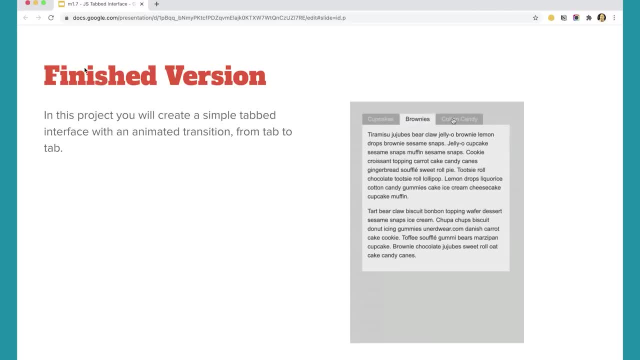 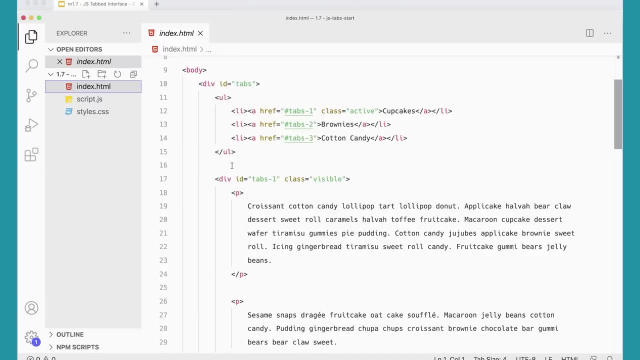 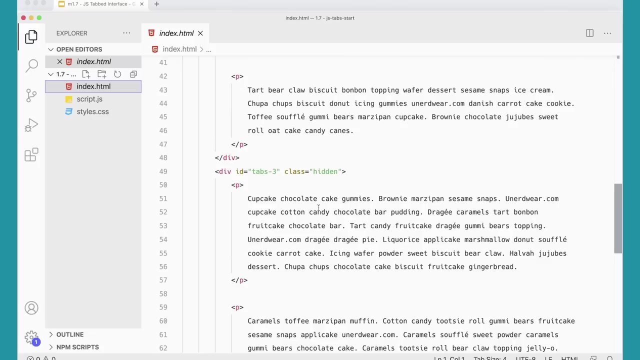 except now we're going to be using plain JavaScript. to get started, I have my files open in Visual Studio Code and you can notice that it's a little bit different in the setup. and then I've added these classes- class visible, class hidden here- and we're going to 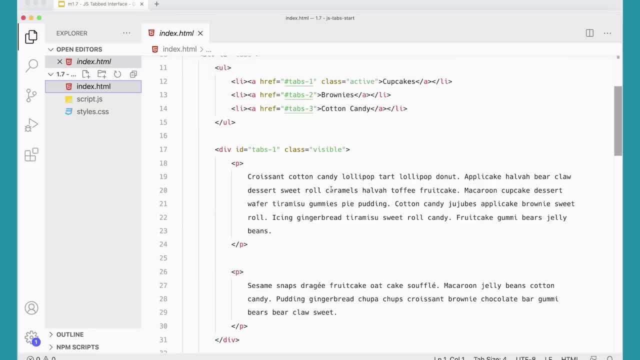 basically be making use of classes because we don't have the, we don't have the jQuery effects library at our disposal. we're going to have to make use of CSS in classes to do the animation and do the hiding and showing things, and we'll use JavaScript to 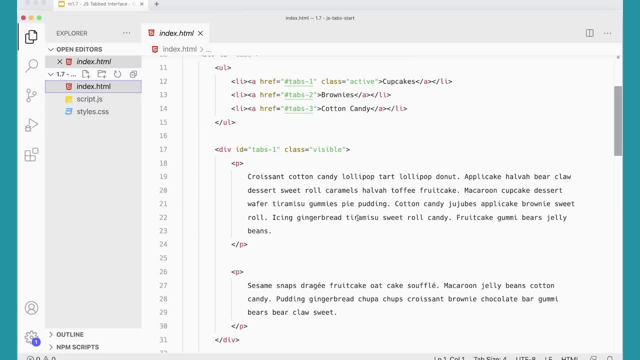 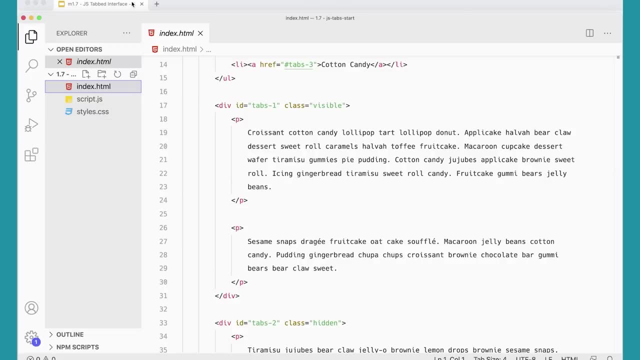 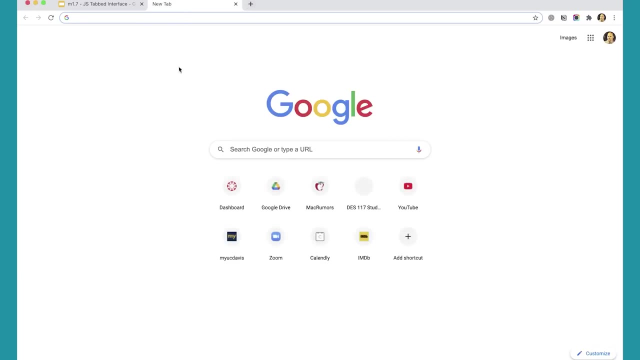 trigger the changing of these classes. so we've got these pieces here and then the first thing we're going to need to do is work on our CSS a little bit. well, first, over here, I should open up this file here. so I'm just going to make a new tab and open. 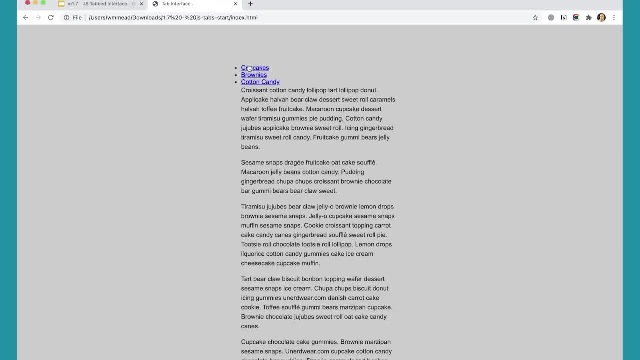 this file. you can see that it looks the same as the previous one. I've added a little bit of the styling here already, but the first thing we need to do is get these things styled, and the styling for getting these things styled is exactly the same that we did for. 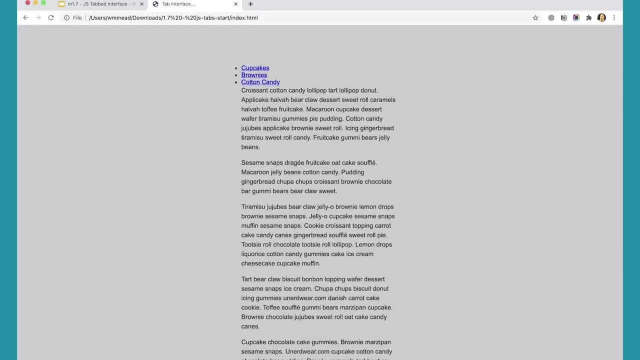 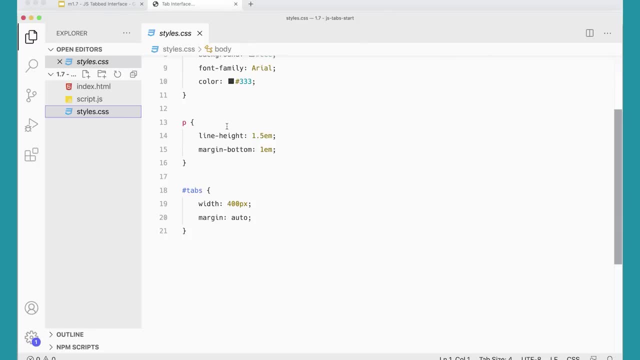 the jQuery tabs so you could actually go to that project and get that same styling from there. but over here I'm just going to come in and just add, I'm just going to paste it in here. but this is the exact same rules from the previous version we're setting. 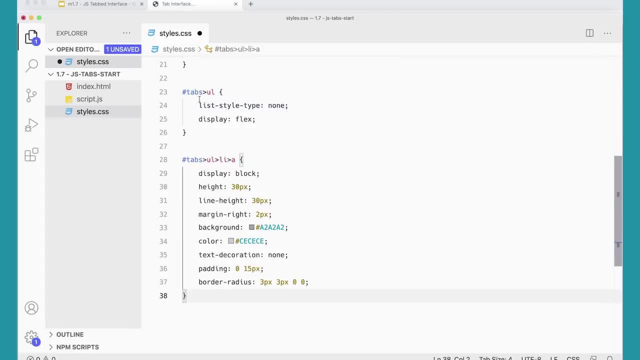 the for the unordered list inside the tabs and we're using the anchor bracket because we want to target those elements specifically and we're setting them to display flex so they go next to each other and then down here from the anchor tags, we're setting them to display block. 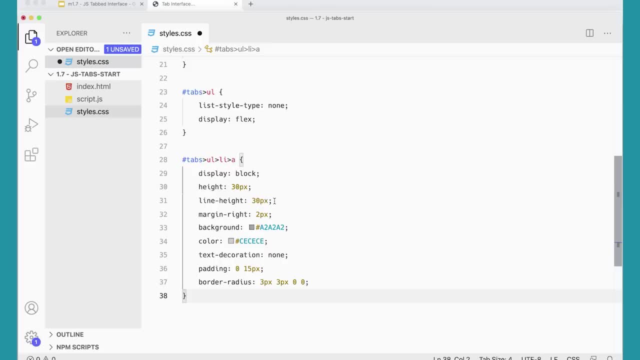 height: 30 pixels. line height: 30 pixels, which puts the text in the vertical center margin on the right 2 pixels, and setting the background color, and all that stuff is exactly the same, along with the border radius and all that, so that should all work to get. 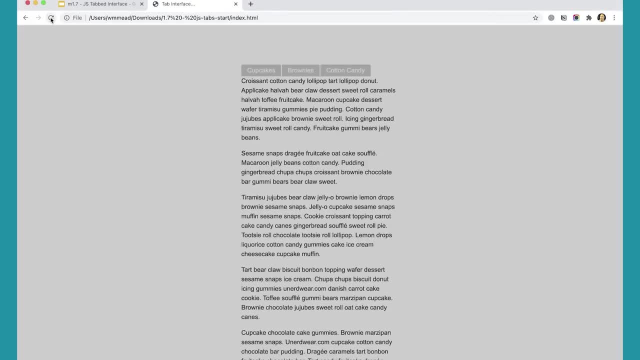 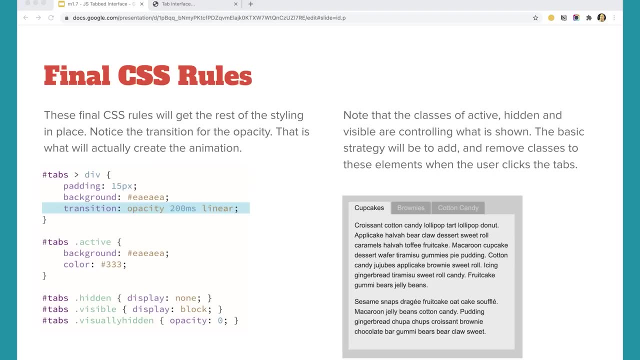 our basic tabs to look the way we want them to look on our design, and that's really critical to kind of get started with there. the rest of the styling that we need is a little bit different, and basically what we're doing here is I'm making these divs. 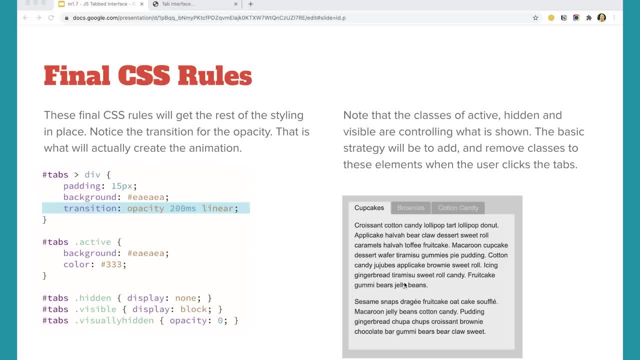 that's these divs down here. they're going to be set with padding, 15 pixels and a background color that's that lighter gray, and then the transition is what's going to actually handle the fading in and fading out of the opacity, and we'll see how that works in the script. 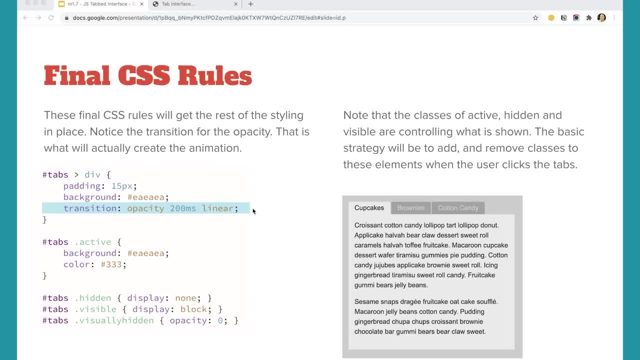 but this is where the actual animation is going to take place- is here in CSS, so that's a little bit different. then I have a class of active on the current tab up here that's selected and that's going to get the background color that matches that background. 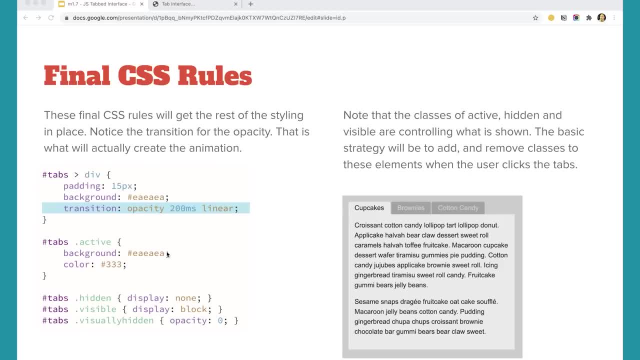 color and the color of the text and you can see over on the HTML if you go. look that the current tab, cupcakes, is active. it has the class active on here. so in our JavaScript we'll be moving that class active to each of these. we'll be moving it from here and adding: 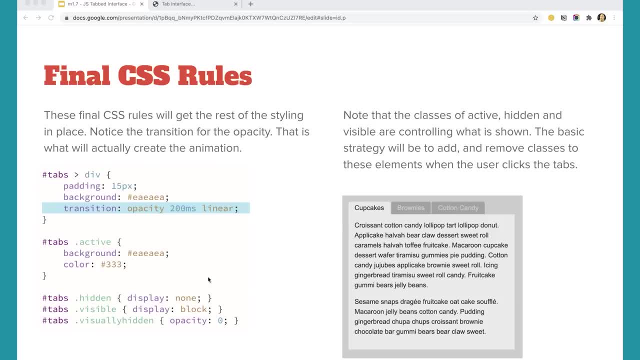 to each of these as you click on them to change them. and then we've got a few helper classes down here that we'll be using: hidden to set elements to display visible to display block, and visually hidden, which is going to be the opacity, and that's where it gets animated down. 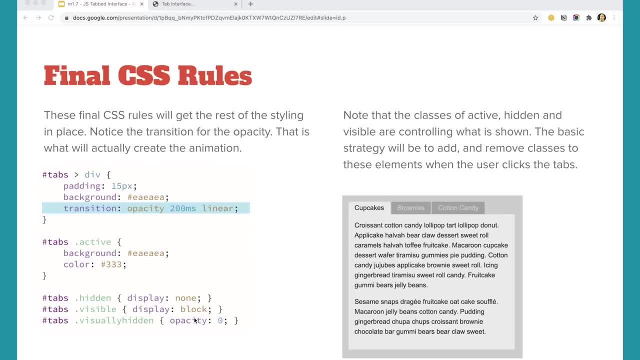 so you'll see how this all works in the JavaScript, but for right now we need to add this over onto our CSS and you're going to have to type it in. I'm going to paste it, so you don't have to watch me type it, because it's not that interesting to watch me type. 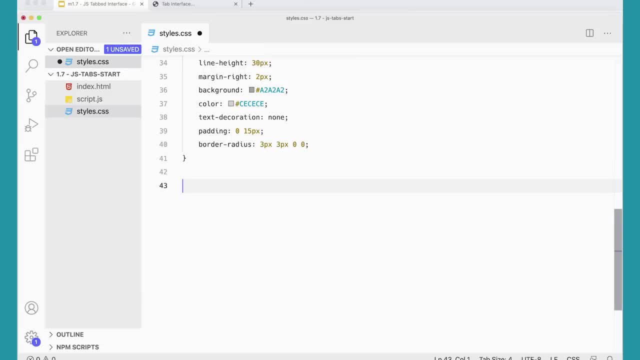 this, but I'm going to paste it in here. but you can pause the video and go in and add this yourself. so just pause the video here and add these rules on your CSS tabs. angle bracket div. set the padding to 15 pixels, the background color and. 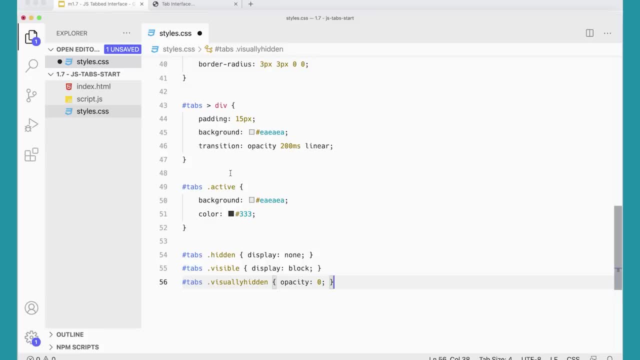 transition. we're going to be transitioning the opacity over 200 milliseconds in a linear using linear easing, so it's going to be the same speed all the way through. and then the active class on the tabs gets its background color and the color. and then we need these three little helper rules. 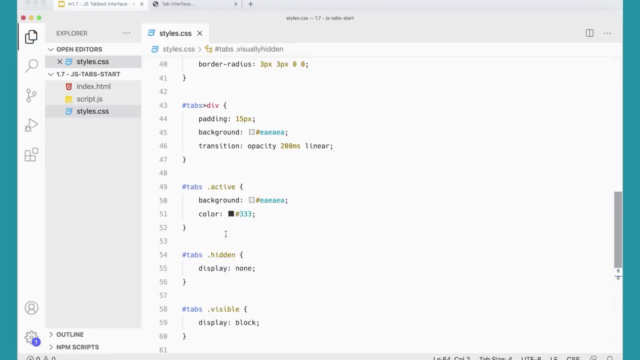 down at the bottom here. so I'm going to save that. and of course Visual Studio Code likes to have them slanted this way. I kind of prefer these all in one line myself, because they're just one declaration each. it's a little easier to read. but that's okay, we'll let Visual Studio 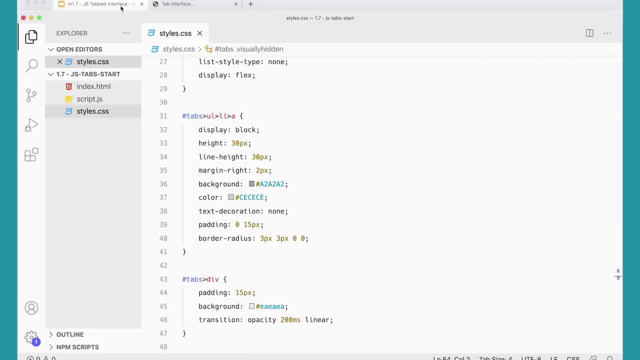 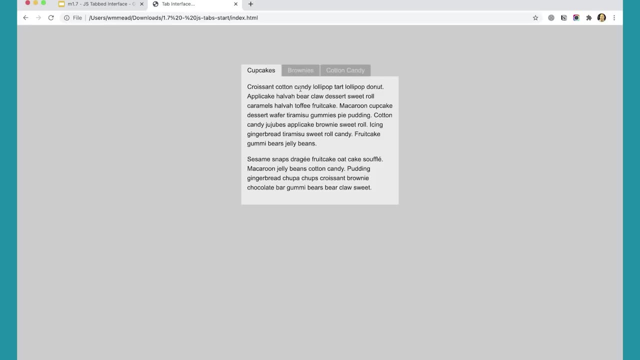 Code have its way with it. okay, great, so now we should have the look that we need for our tabs. if I come over here and refresh, it looks just like it did before. none of this is actually functioning yet, but the look is the same as what we 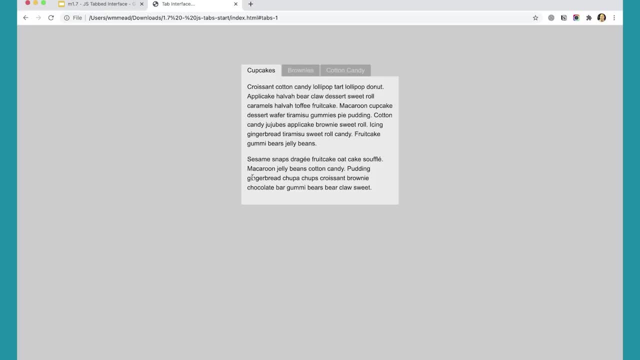 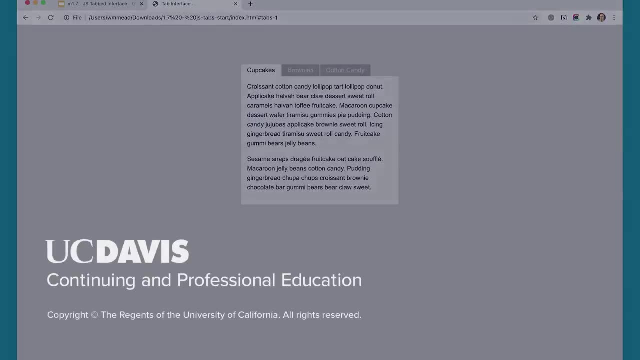 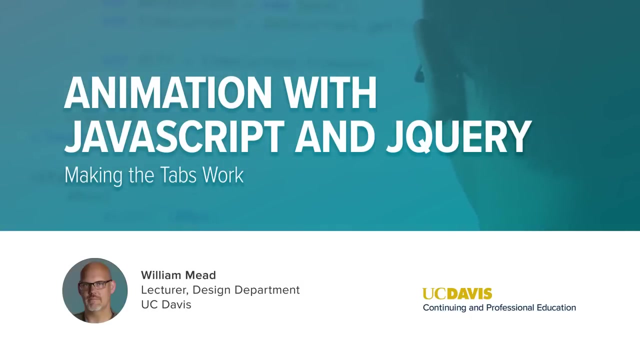 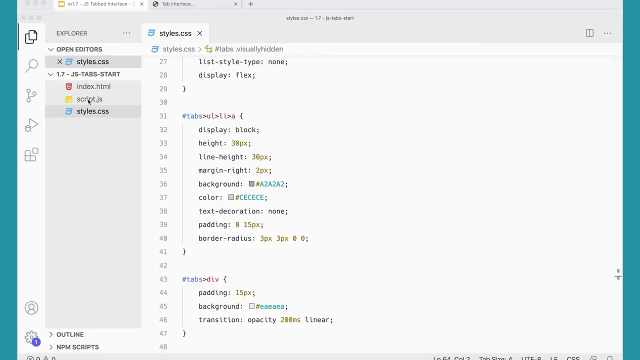 had in the original, in the original version of the jQuery version, and we'll start working on the JavaScript in the next video. hopefully you got all the CSS in place and now you're ready to start working on the JavaScript, and I have a linked script file here and it's linked at the bottom. 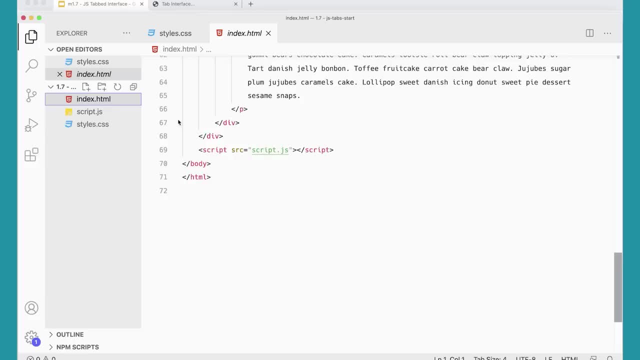 of this file. you can see down here. I've got my script file in, so I'm going to go to that script file and just work directly in here. I'm going to just use var for right now and later go in and clean up with and add, let and const. 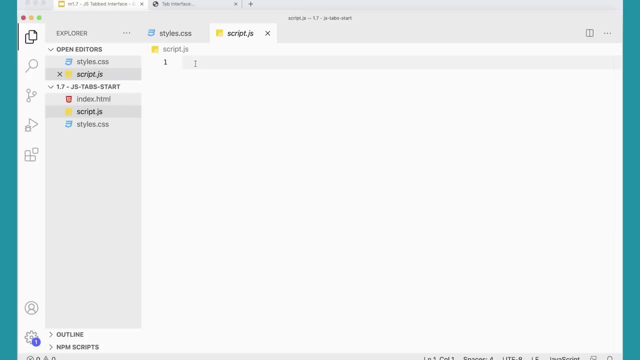 and do that kind of stuff. but you could use let and const right from the beginning here. but the first thing I want to do is get all of my tabs and put them in a variable. so I'm going to make a variable var tabs and set that equal. 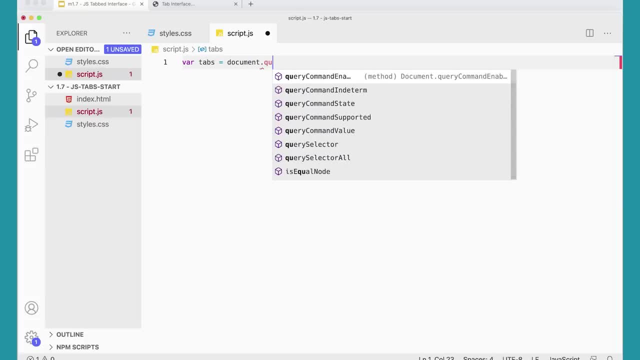 to document dot query selector. all and what do I want to get in here? I want to get very specifically the pound tabs, angle bracket, ul angle bracket, li angle bracket, those elements. these are the elements that I want to get and assign to my tabs variable. then I want to add: 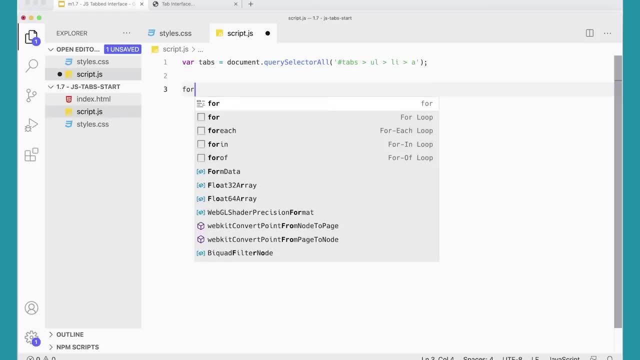 a click handler to all of them. so I'm going to use a loop, for var i equals zero, var i is less than tabs dot length i plus plus curly brace. and then down here I'm going to say: okay, tabs, square bracket i, so each tab as we go through this loop. 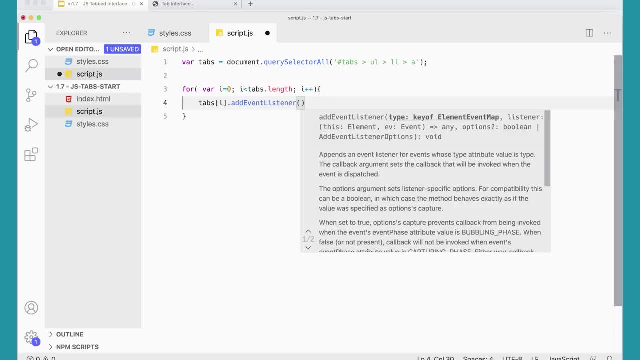 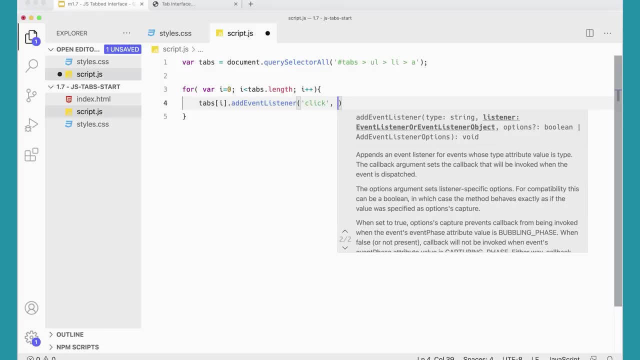 I'm going to add an event listener and the event listener is going to listen for a click right and then, when the click happens, we're going to run. we could run a function and we could do an anonymous function like this and put everything inside of here. 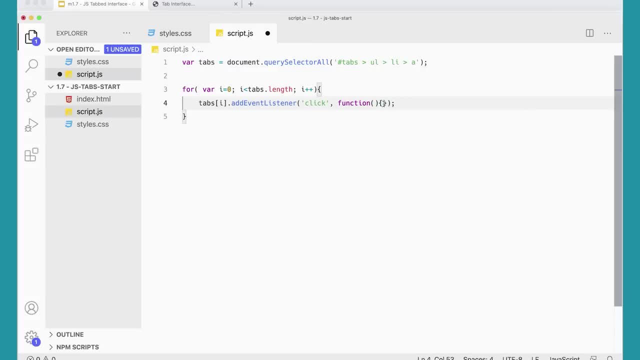 but in this case I think it will be a little bit cleaner to make a separate function. so I'm going to have a function down here: function select tab or select tabs. I forget what I did. I'll leave it select tab and parentheses curly braces. so instead of an anonymous function, 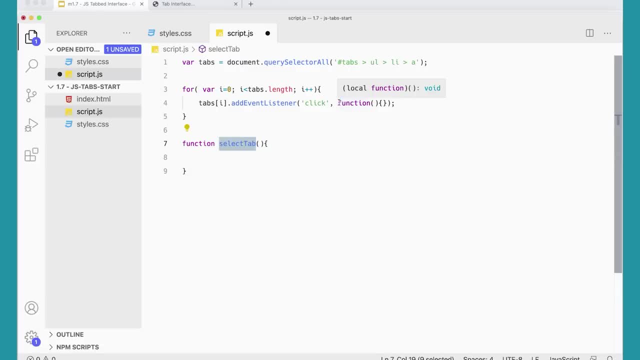 I'm going to run select tab, so I can just copy that instead of here. when you do this, you don't put in the parentheses up here. if you put in the parentheses, it will run right away, and I don't want it to run right away. I want it to run when I click on this thing. 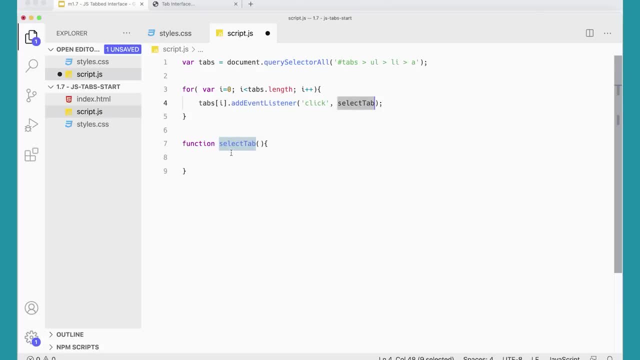 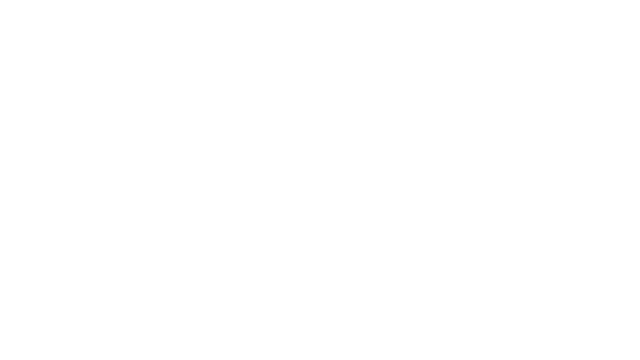 so I just put the name of this function here and that will run this function. so that's going to get us started with getting our tabs, and then we need to. the next thing we need to do is figure out what we need to do in here. so what do we need to do in here? 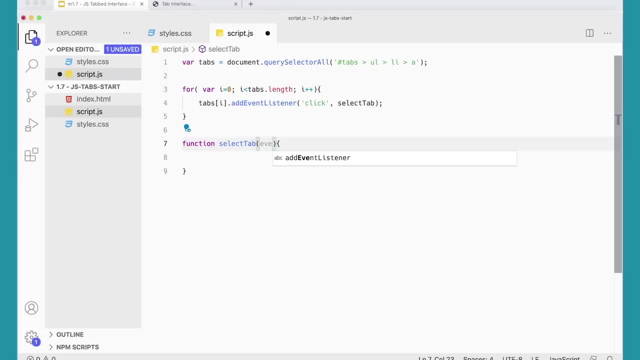 well, the first thing I'm going to do is I'm going to pass in the event object here so I can do eventpreventDefault, and what that will do is make it so that when you click on the tabs over here, you don't get the little hash showing up at the end of the 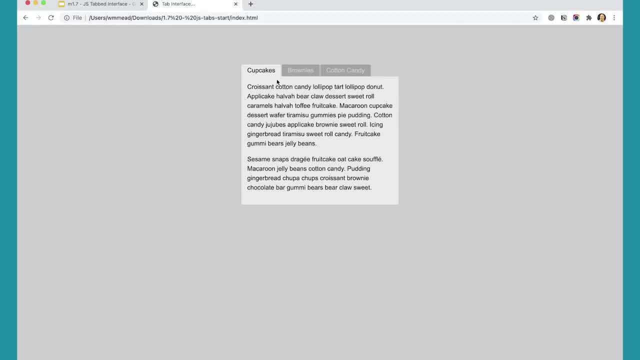 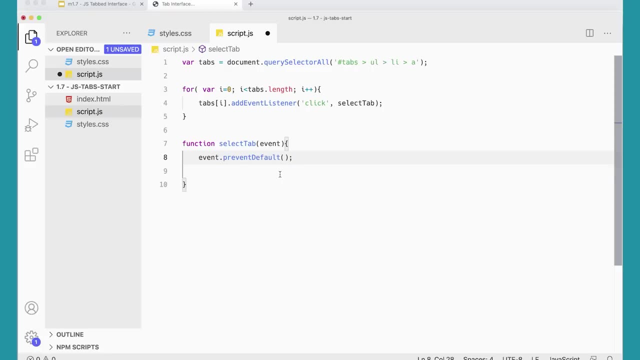 URL. I don't really want that to happen, so so preventDefault will keep that hash from showing up when I do that. so that's great. and then I need a little bit of a loop. I'm going to just do a forward loop and basically what I 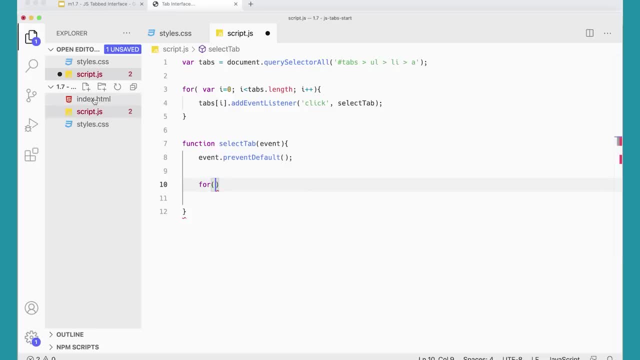 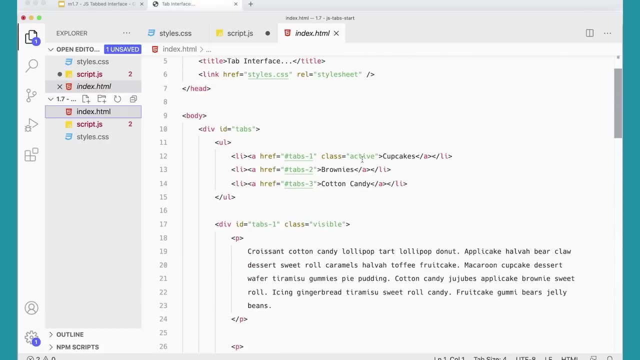 want to do is: I want to go through and remove on index. I want to remove any class that's on any of these links, so this one has the class of active on it. I want to remove the class of active from all of these and then add it to the one. 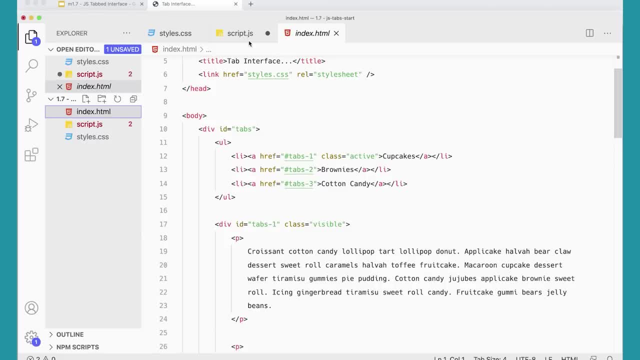 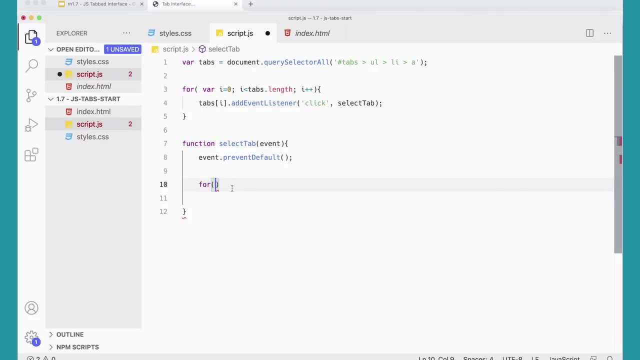 that I clicked so it gets the correct class on there. so I'm going to use a loop to do that. in jQuery we didn't really need to use loops because we could apply things to groups of elements using the jQuery object, but in plain JavaScript we need to loop through and do this. 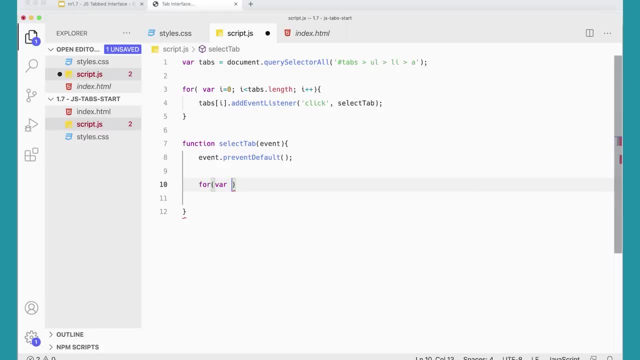 so here I'm going to add bar: i equals zero, while i is less than tabs dot length. we're using the same variable that we created up here: global scope there. and then i plus, plus, and then I'm just going to go through and say, okay, tabs. 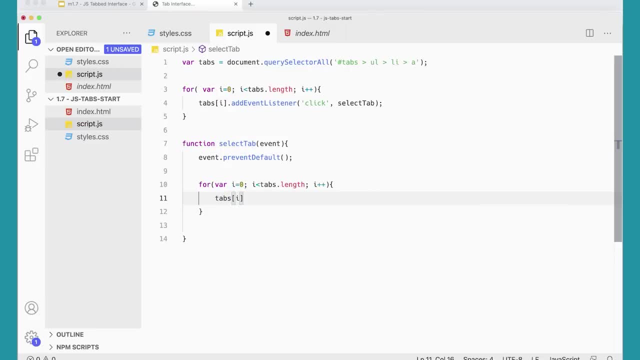 square bracket, i dot remove attribute- remove attribute. there it is: remove attribute class and that will remove the class attribute from each tab. that will get rid of all the class attributes. then, after I'm done with that loop, I want to add it to the one that I clicked on and I could use. 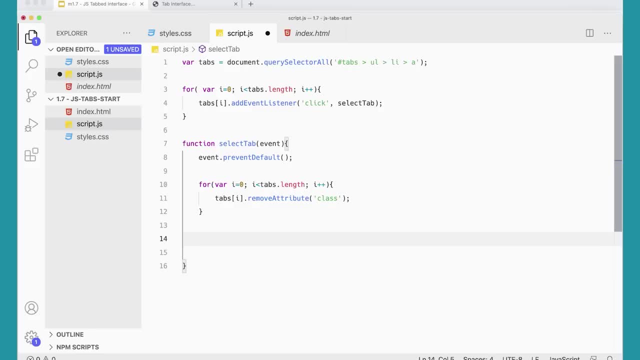 this keyword here, but I think it's a little bit easier and better to use the event object that I've already passed in and used with event prevent default. you can use it again here: event dot target. that will get this item: event dot target, dot class name. 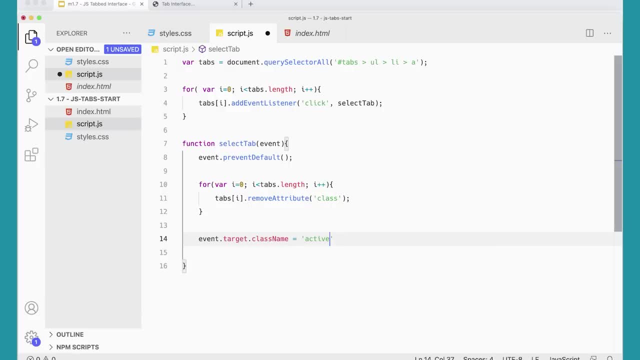 equals active and that will put the active class on the one that I clicked. so I'm removing it from all of them and then putting it on the one that I clicked. so what we did in one line of jQuery, we're writing a little function here to do in plain javascript. 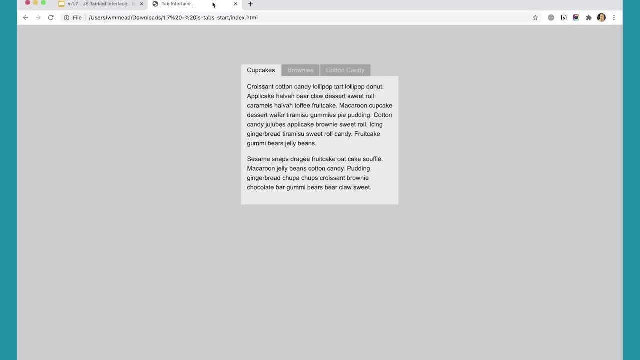 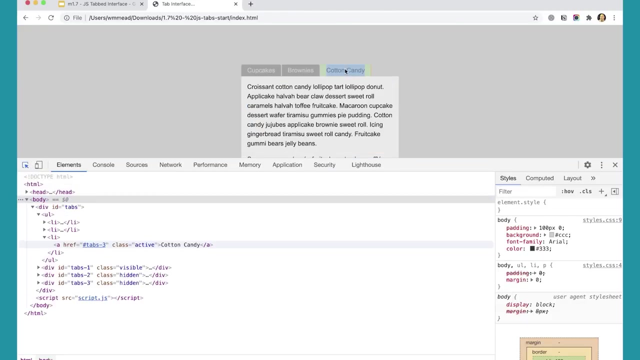 but that should work. let's go over and test it. if I refresh this and click brownies, you can see it's getting the correct class on there, and if I inspect and look at my elements here, you can see that one has the class of active on it. 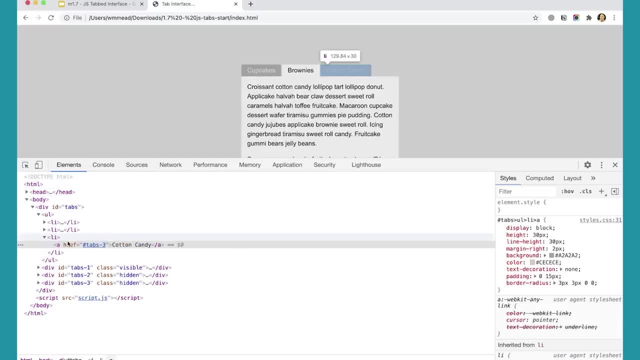 but then when I click on these, that class goes away on that one. but now it's been added here so that one has class of active and we can see it moving around that class active is moving around to each one of these. okay, great, so we've done half our project. 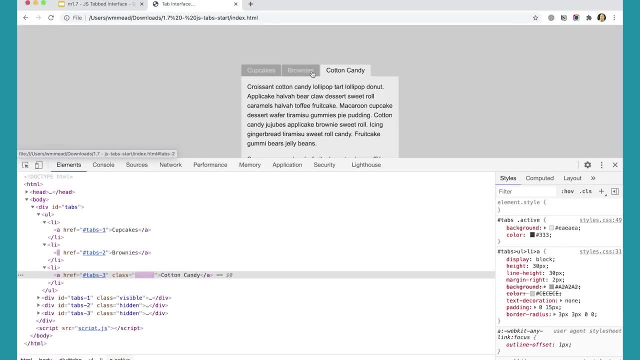 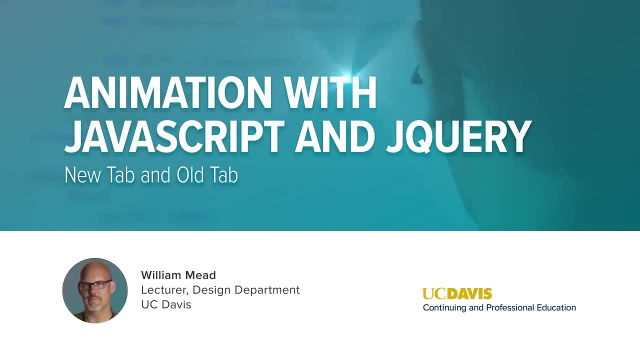 we've made it so that you can click on these tabs and have the correct classes, and it looks like it's doing that. now we have to actually make the content work, and we'll do that in the next video. now that we have the actual tabs working properly, we have to. 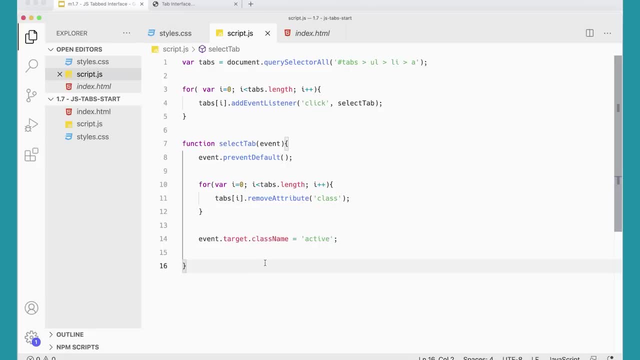 do something with our actual tab content to get it displayed. we have to do something with the new tab that we clicked on and the old tab that is going to go away, so we're going to do that here. the first thing we're going to do is we're going to 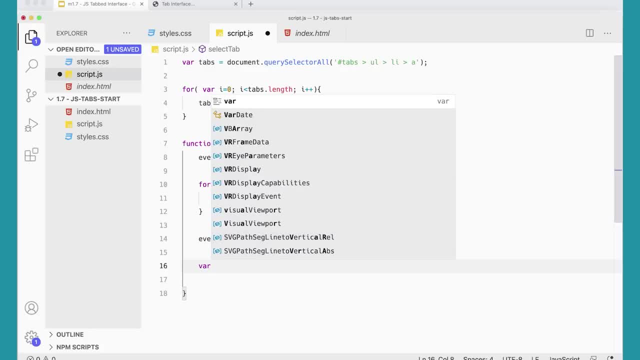 make a variable here, var this tab, and we're going to make that equal to event dot target- again the one that we clicked on event dot target, dot get attribute and we want to get the href attribute, so that will get the href of the link that we clicked and 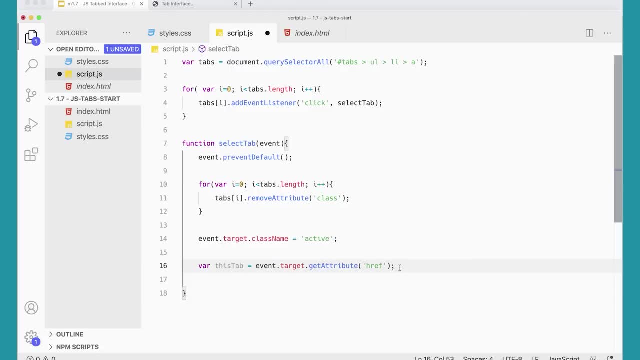 put it into this tab, okay, and then we want to actually go and get that element, so I'm going to have another variable, var- this content, and that's going to be equals document dot. query selector- query selector: this tab, because we know that this tab is going to return the href. 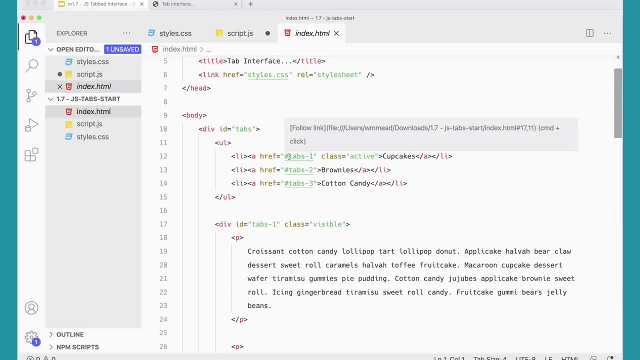 attribute is going to return either a pound tab dash one or a pound tab dash two, and then so we want to go get that div for whichever one is clicked, and again only one of these can be clicked. so if you click on brownies, it's going to get the class active. 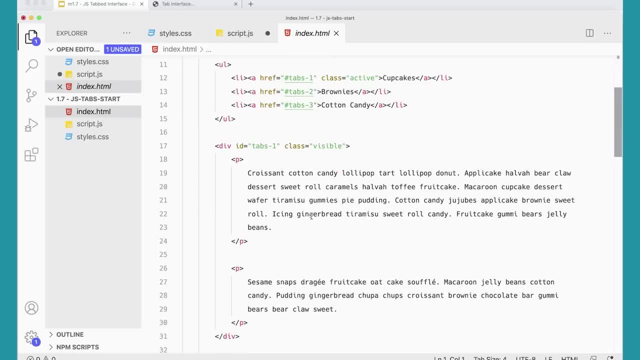 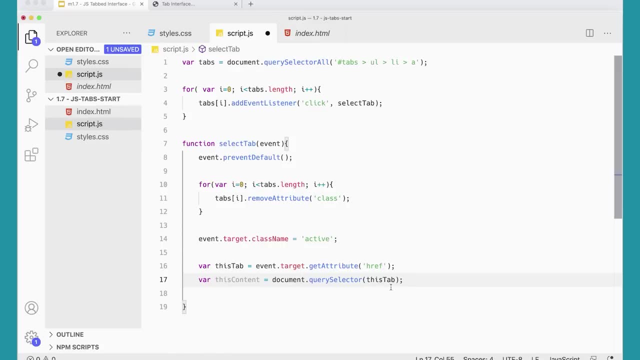 then we're going to say, okay, go get tabs two, and that's going to be this one down here. so that's what's going to happen there: to go get those two things. so we've got those two things and we're going to just hold off on those for a 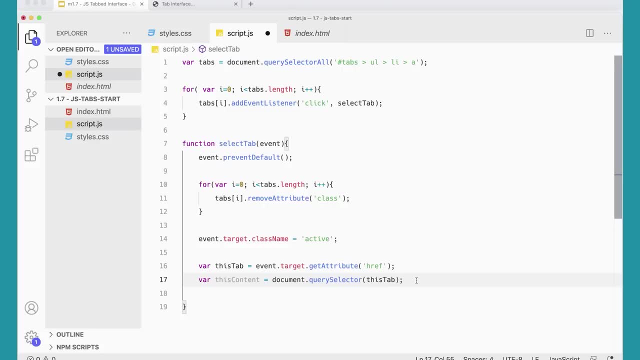 minute and let them do their own thing in a minute. but now we need to do something with the old tab and get its content. get its content. so we know what we're going to do with that one. so here's what we will do. we will add another. 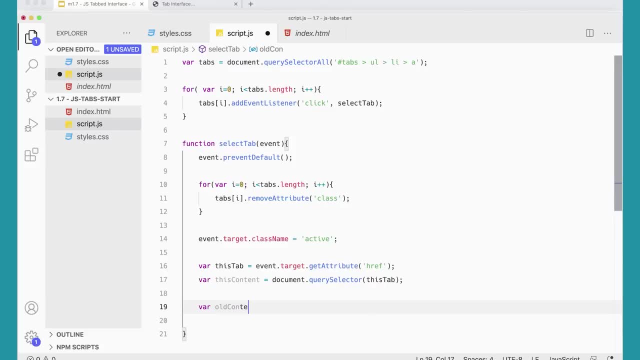 variable var old content. and I'm going to have that equal document, dot query selector quote: single quotes there: dot visible. now in jquery we have the colon visible filter. that would get visible tabs. but here, since we're not using jquery, what we're doing in jquery instead is each of. 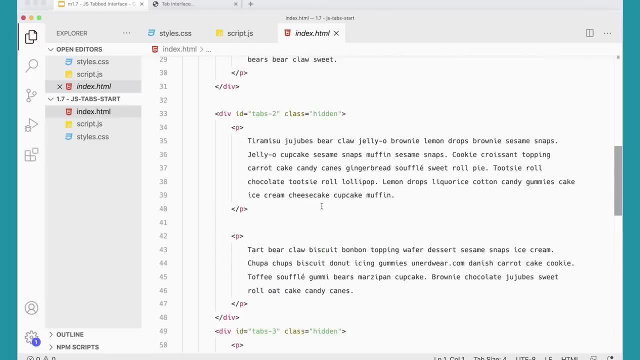 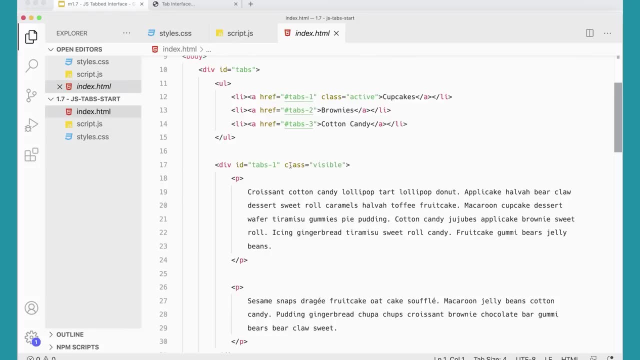 these tabs has a class of either hidden or visible on it, so the one that's visible. so, basically, what we're going to do is we're going to swap these classes around so that when we click on one of the tabs, this one's visible, we'll get this one, and that's. 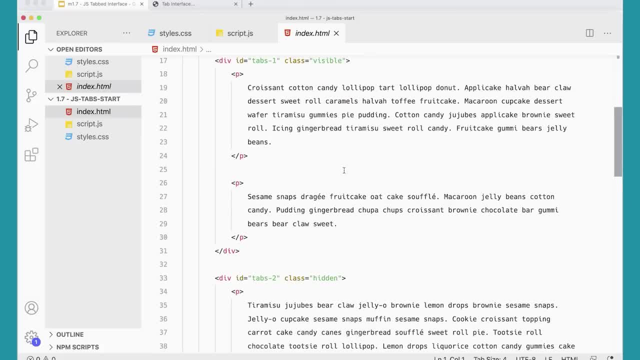 going to be the old one and we're going to change it to hidden while the other ones become visible. but we have to do kind of an intermediary step to get the animation fading in and fading out. that we'll take a look at and see how that works, okay. 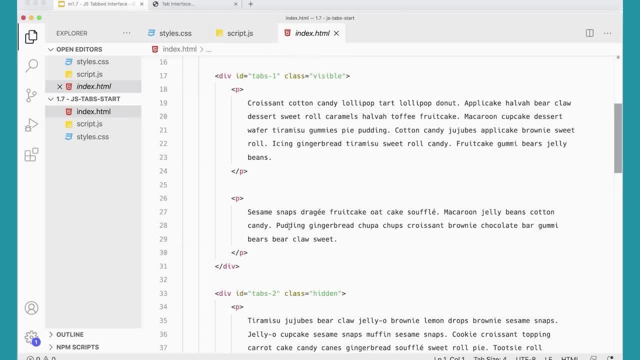 but essentially that's what we're going to do is we're going to get those elements and work with that. now that we've got this element- the one that we the old one- what we're going to do is we're going to set its class name to visually. 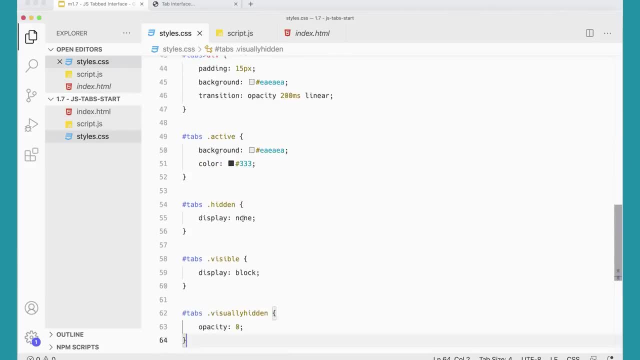 hidden and over here in our styles, we remember that visually hidden will set its opacity to zero and that will trigger this animation which changes the opacity down to zero over 200 milliseconds. that will actually fade it out when we do that. so over here we're going to do. 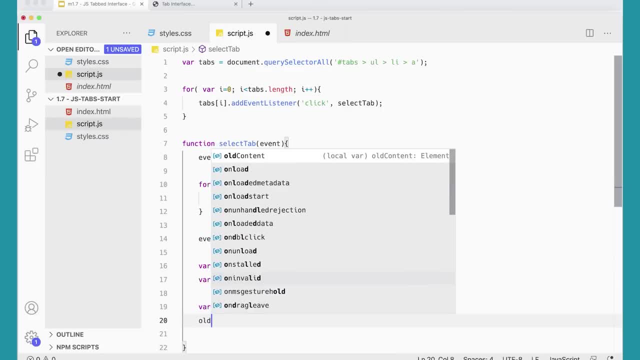 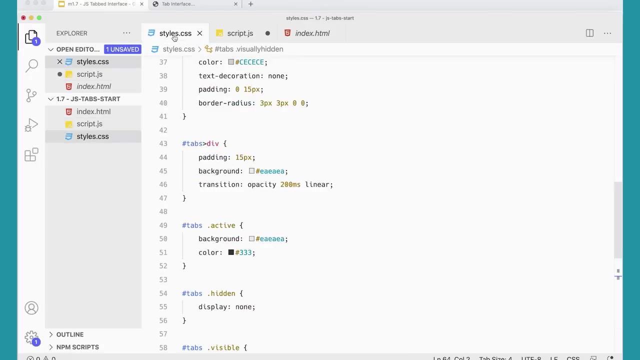 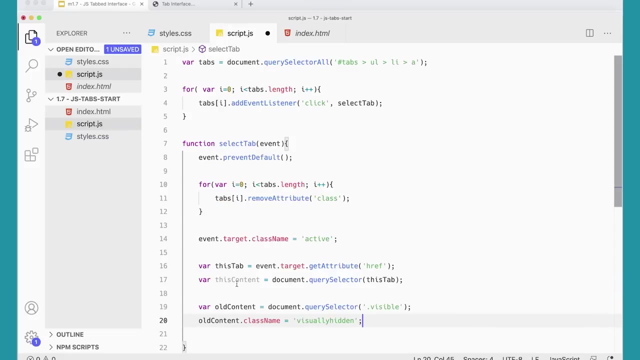 old content. old content dot. class name equals quote: visually hidden. make sure it matches how you spell visually hidden over here. i'm just going to check and make sure. yeah, just do it all over case one word: visually hidden. so that's going to, that's going to set. 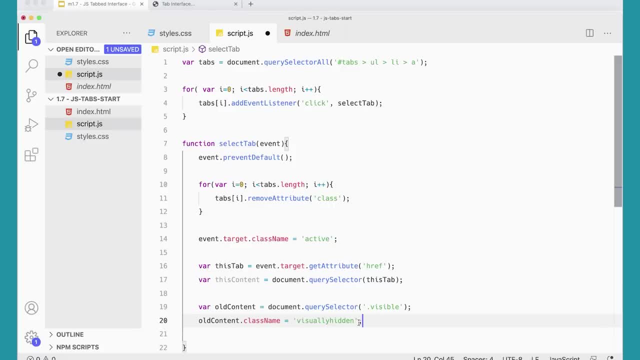 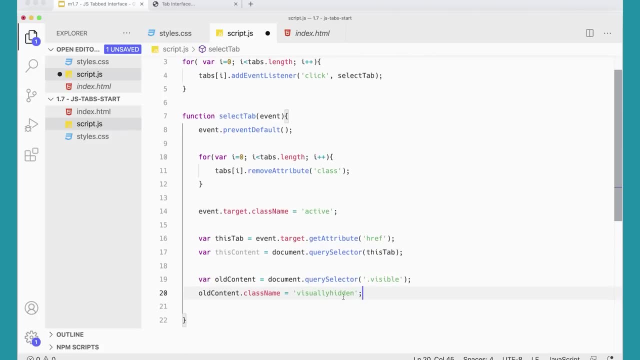 that one to visually hidden. so that's going to trigger that animation and hide it while it's um, while it's um, while it's on the screen there it'll run for 200 milliseconds and visually set it down to opacity zero. it's still on the screen, but it's just it's. 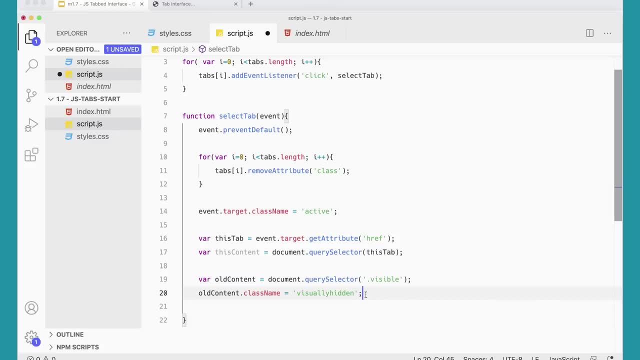 just been transitioned down to the opacity zero, so you can't see it anymore. so, then, what we need to do is we actually need to add an event listener to this old content, and when that animation, that transition has finished, we need to do something with it. we're going to take it off. we're 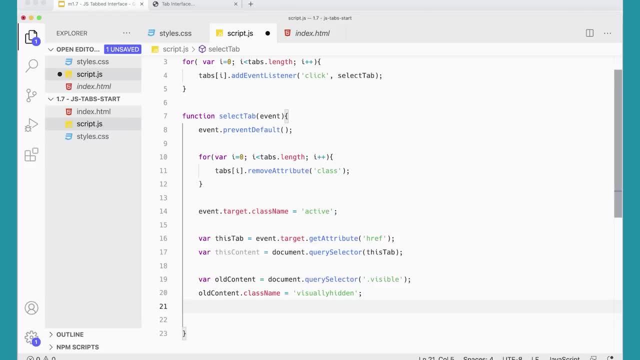 going to set it back to its basically displaying none at that point, and so in jquery we have these great callback functions after the effects library does its effects that we can use, but here we don't have that. instead, what we're going to use is an event listener, so i'm going to 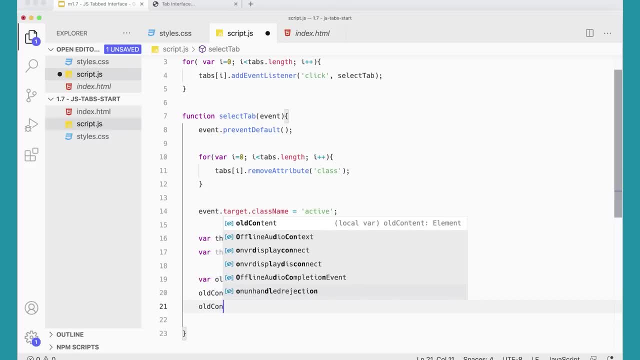 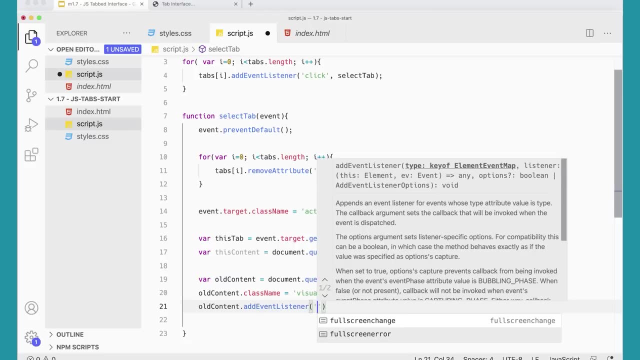 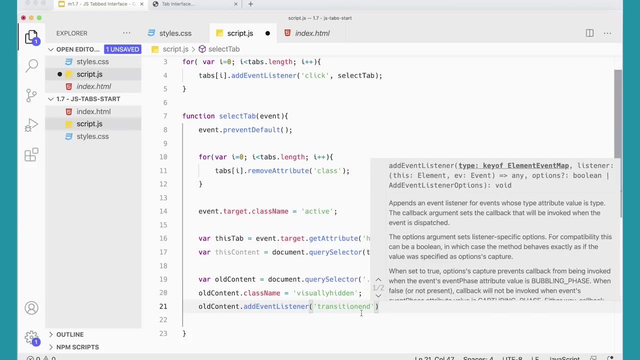 put an event listener on old content. add event listener. and the event that we're going to look listen for is transition and- and this is be sure you get this right- transition and it's not transitioned, it's transition and the end of the transition. make sure you get that right, because 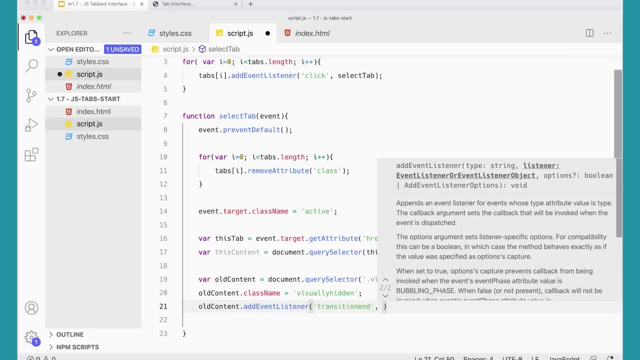 when i've done this assignment with students in the past, it's frequently where things go wrong. people put transition, which kind of makes sense, but it's actually transitioning okay. so once this content, it has the transition has ended. so transition and we're listening for that end of that css transition. it's. 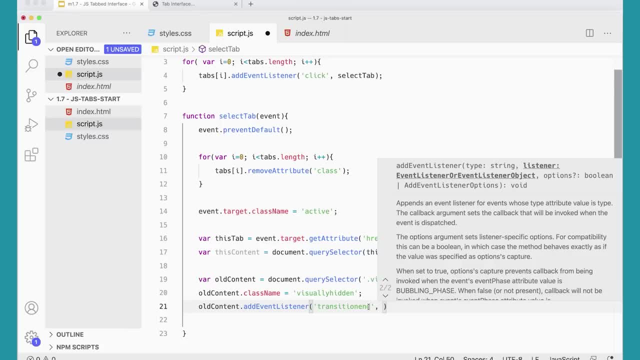 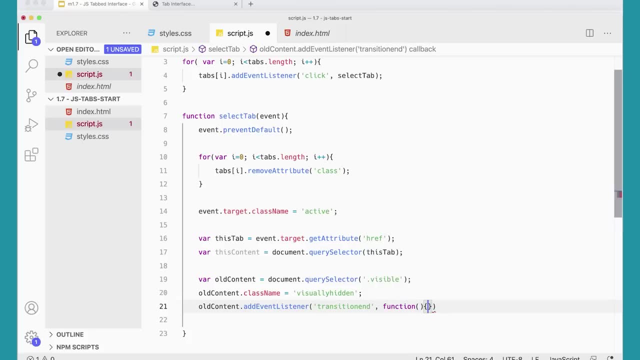 pretty cool that we can do this in javascript is the end of a transition, a css transition. we're going to run a function that's curly braces and a semicolon and in this function we're just going to set the class name on this to you know. 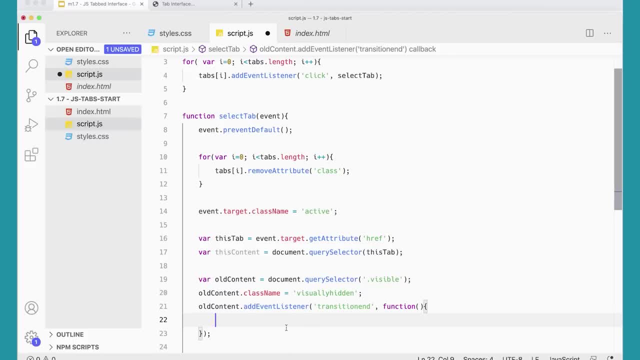 after it's transitioned so that it's invisible. we're just going to set the class name old content. that class name equals hidden, because now we can just say display block none. we've transitioned it down to opacity zero, now we can just set it so display none instead. 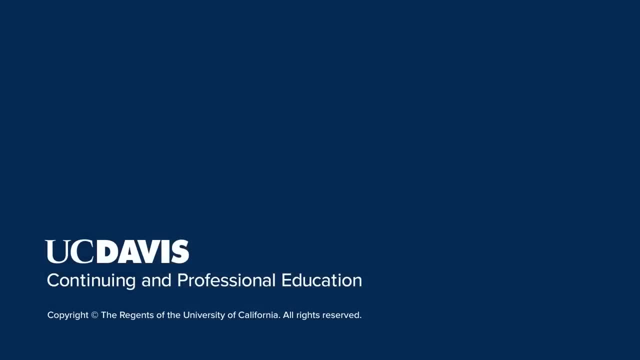 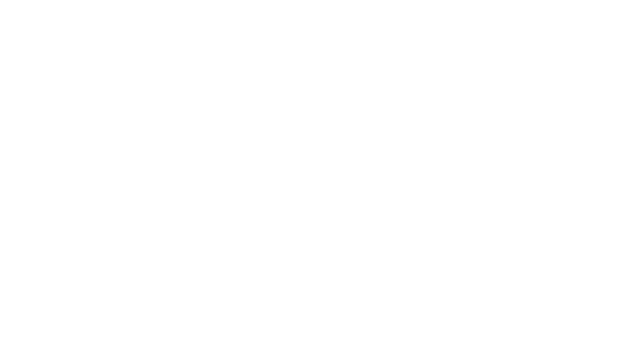 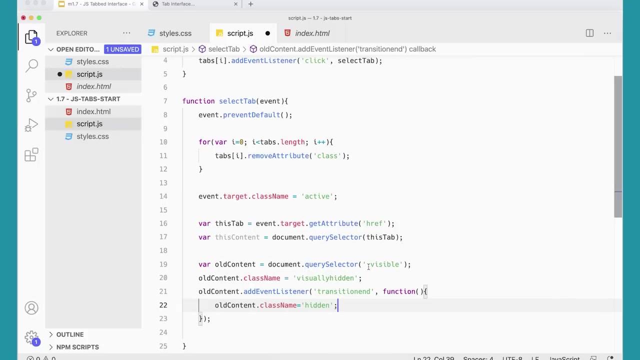 of display block at that point. we've taken care of the old content so that we've set it. we've taken the old content- what was the element that had visible on it? and we've set its class name to visually hidden and that fades it out, that sets it down, so its opacity. 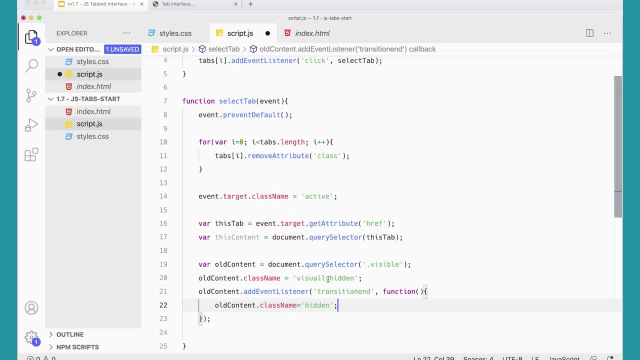 is at zero over 200 milliseconds. when that transition has ended, we're going to run a function to set it so that it's completely hidden, and that just sets it to display none, so that it's off the off the dom entirely. now what we want to do is 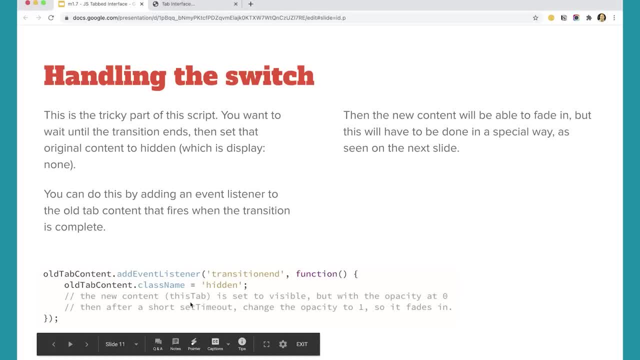 for the new content. we need to handle the new content, which is this tab, the tab that we clicked, and the content that goes with it. we need to set it to be visible, but with the opacity at zero, and then, after a very short set timeout- we'll talk about set timeout in a minute. 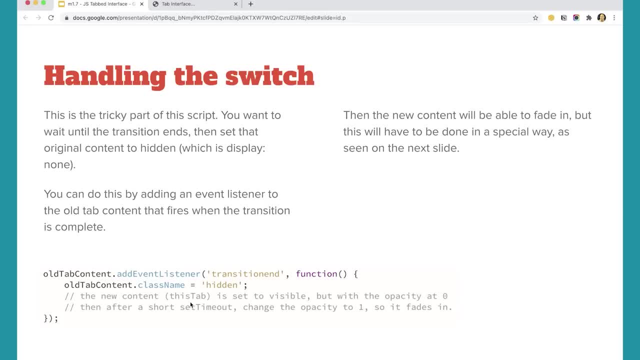 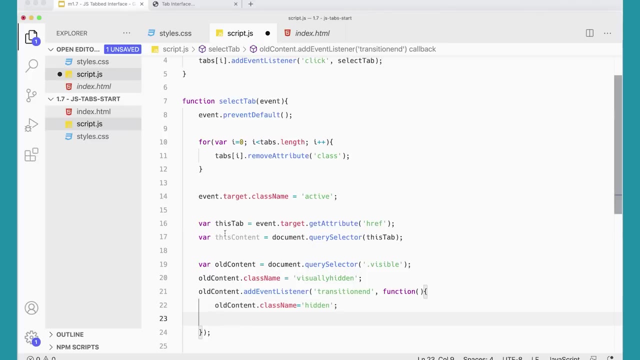 but after a very short wait, we're going to change its opacity to one so that it fades in. so let's do, let's do that really quickly here. so let's do that here. we're going to come down here and we already have a variable, this content- so we can use that. 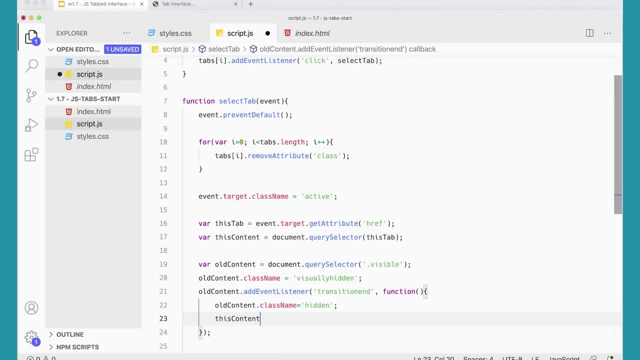 this content. so this is our new content. we're going to set its class name. we're going to give it two classes. we're going to give it the class of visible- visible- I think I spelled that right, hopefully- and visually hidden, and hopefully I spelled that right. 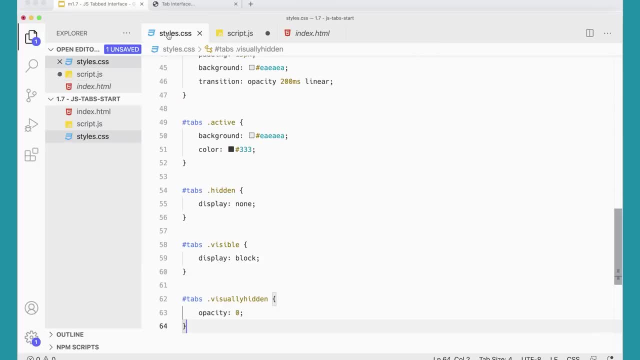 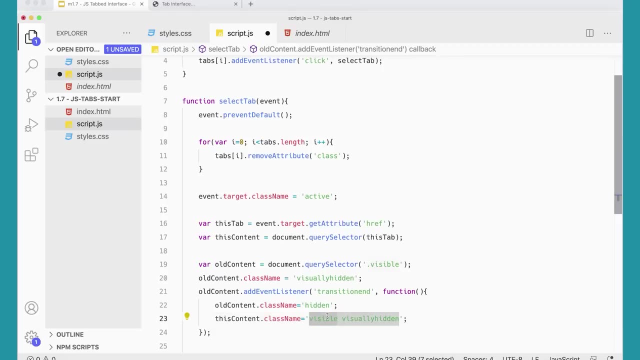 of course you could go over to the styles and make sure you copy and paste and make sure they're spelled right. that's always the best way to make sure your spelling is right. I think I did do it right. and visually hidden, so visible, will set it to display block. 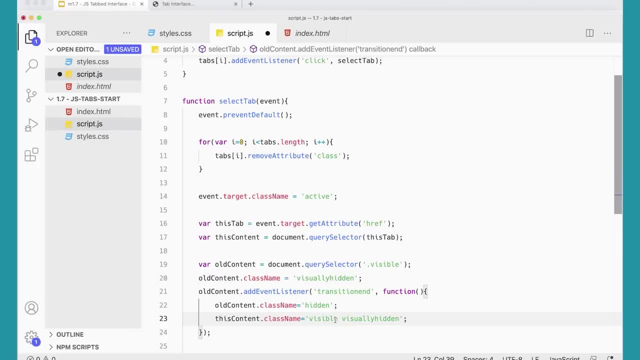 so that it's on the page, but visually hidden will set it so that it's a. the opacity is at zero, and then we need to wait just a split second and then get rid of the visually hidden class so that the opacity comes up to 100%. 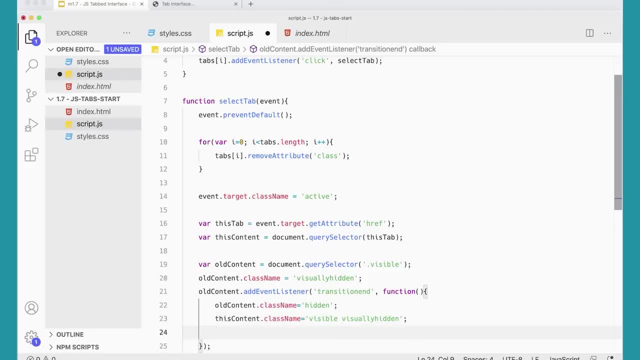 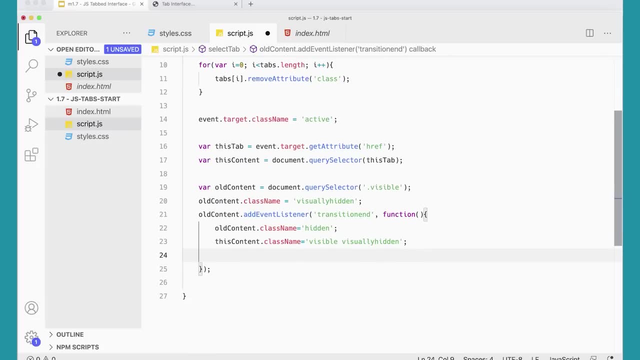 and to make it wait. we're going to use a method in JavaScript that we haven't talked about yet and we'll get more into this in a future lesson, but this is a good place to introduce it. we're going to use setTimeout and setTimeout and we're going to wait a certain amount of time. 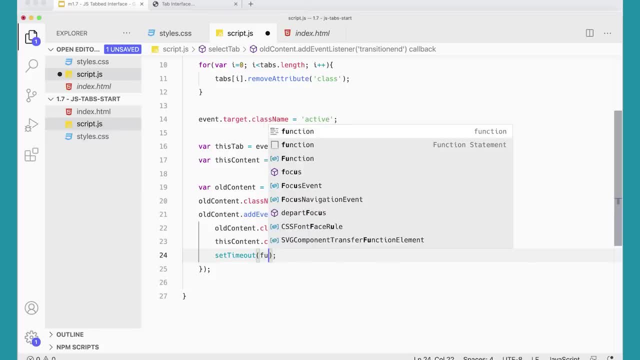 to do something and basically what we can do is we can pass it a function that's going to run over a certain amount of time and I'm just going to wait a split second- like 20 milliseconds, a very short amount of time- just to let that thing come on the page. 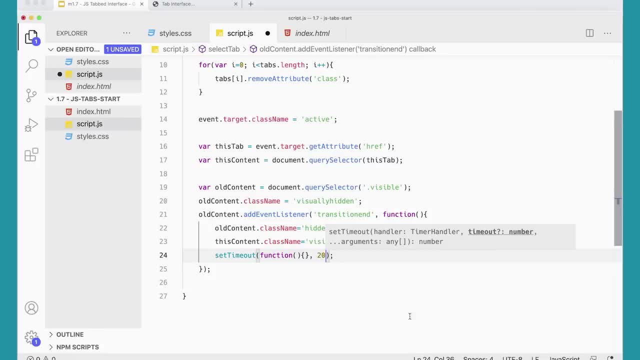 get the class set and then remove the class, so this function will run. this callback function will run after 20 milliseconds. I'm just going to click in the curly braces there. what am I going to do here? I'm going to do this: content dot classList. 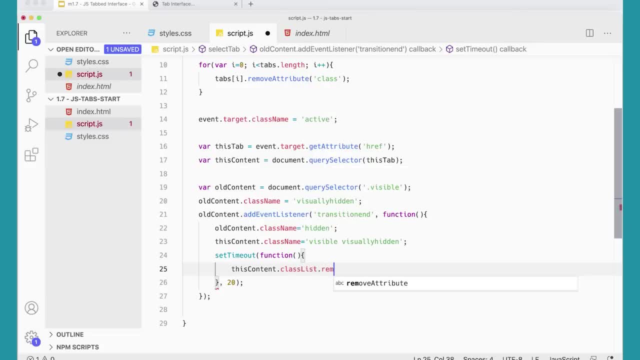 classList dot remove. I think that works. I think I did that right. visuallyHidden- visuallyHidden, visuallyHidden- you can spell that right, so that should wait 20 milliseconds and remove the visuallyHidden class on there. alright, we're ready to give this a try. you'll notice that there's a terrible bug. 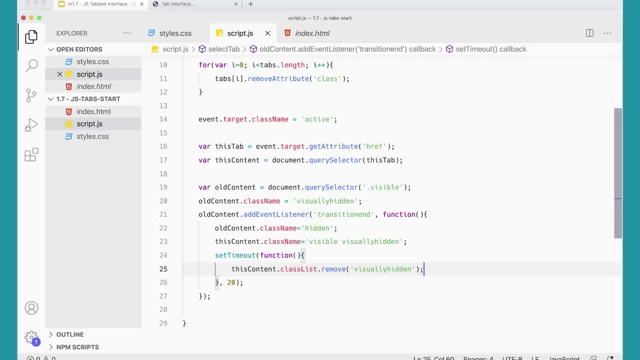 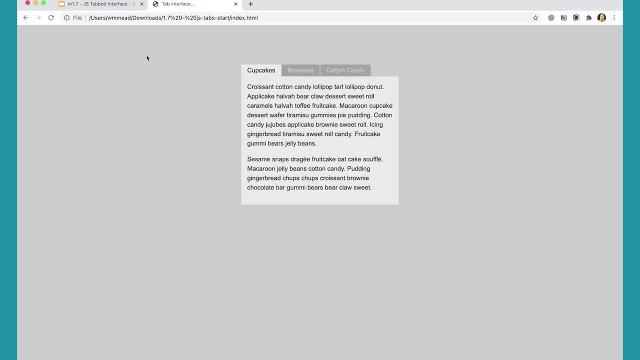 that we need to fix, but it should be mostly working and then we'll fix the bug. so let's give this a try real quick here. I'm going to refresh the page and, if I spelled everything right, it's feeding that one in and switching my tab. 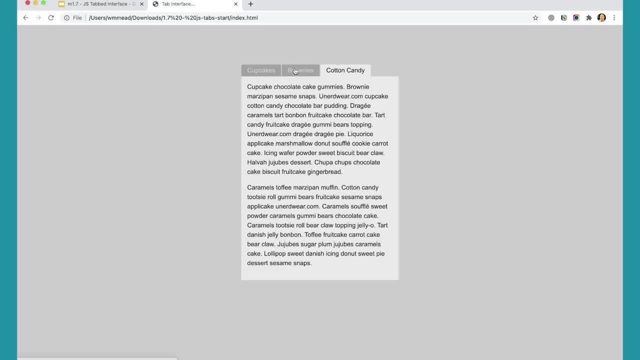 click on that one and it works. it's great. but then, if I click another one again, I start getting this kind of weird thing going on. what the heck is up with that. that is not what I was expecting at all. alright, cool, I'm going to refresh this. 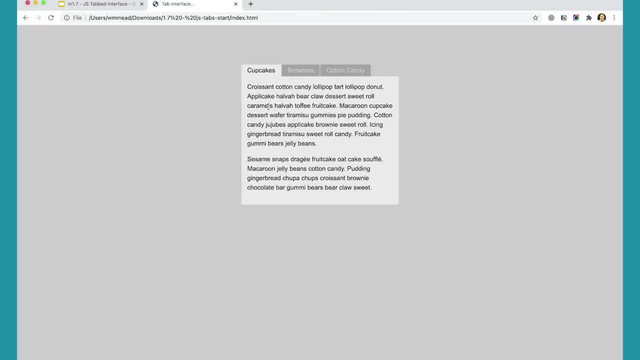 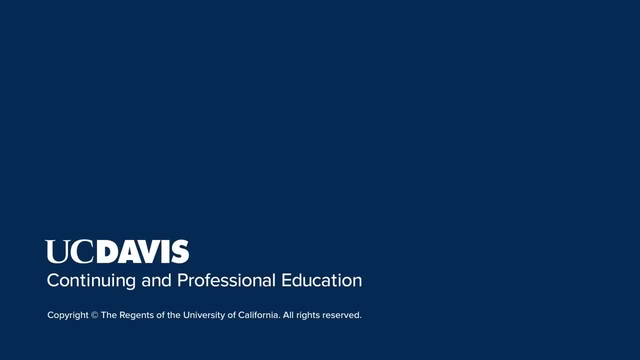 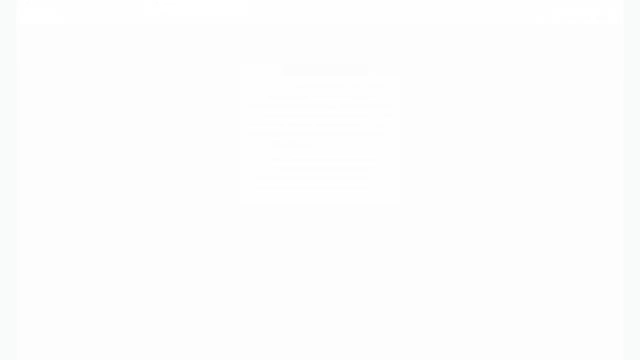 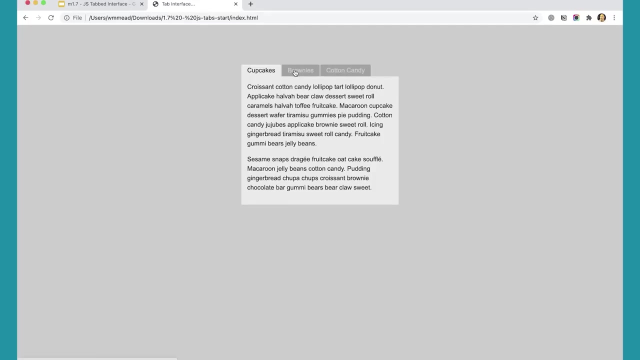 so that I don't have that going on. ok, we're going to fix this and look at sort of the solution for fixing that in the next video. we got our tabbed interface working, but you probably noticed that we had a pretty severe bug where it works once. 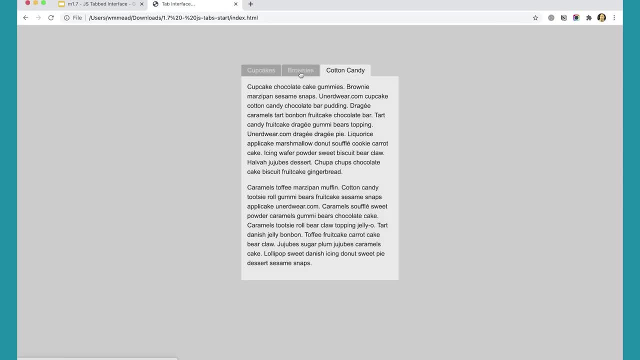 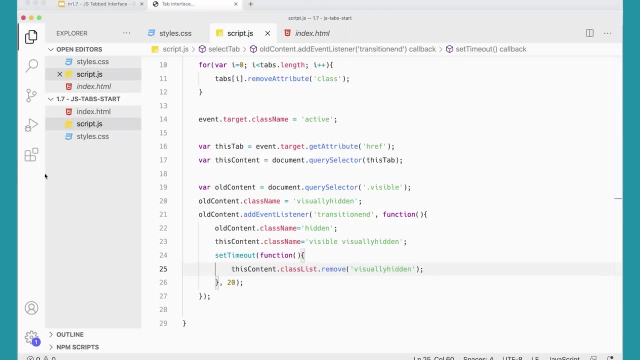 clicking on the tabs, but once we click on them a second time, we get this weird flashing thing going on. so what's going on with that? well, the real problem has to do with this transition end event listener, because we've added the transition end event listener and it works when you click on the links the first time. 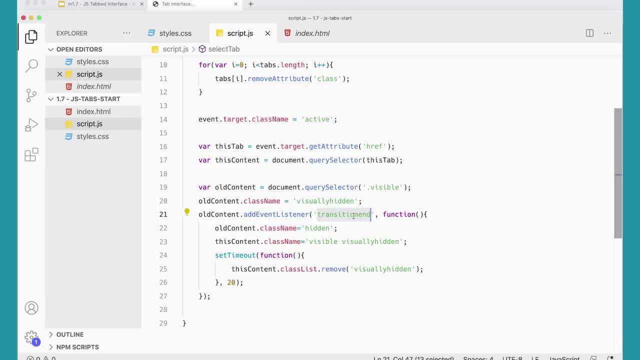 it's looking for that transition end, but that event listener is getting added onto old content each time you click on it. so all of a sudden, when you're clicking on it a second time, it's firing a second time and running again and you end up in this weird loop. 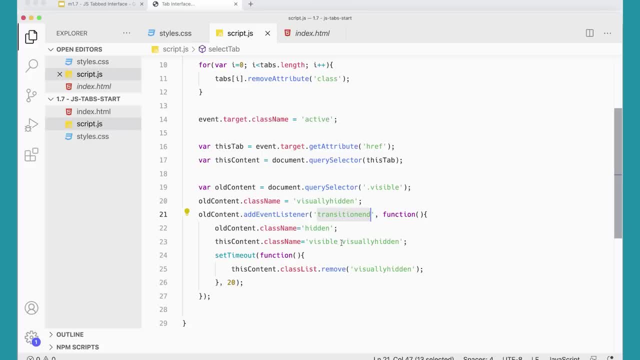 where it's doing this kind of thing. so what do we do about that? what we can do is at the end of this event listener down here after the function. so this function opens here and closes at this curly brace here after this function that runs when the transition ends. 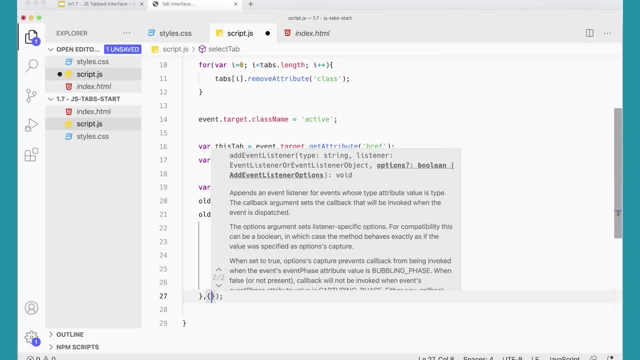 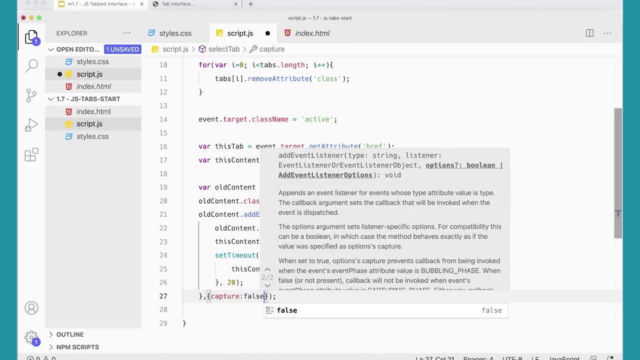 we can put a comma and another object, so another set of curly braces in there and there's actually three settings that we can add to the add event listener. that will help us work with these, with these different pieces here and what they are are capture false once. 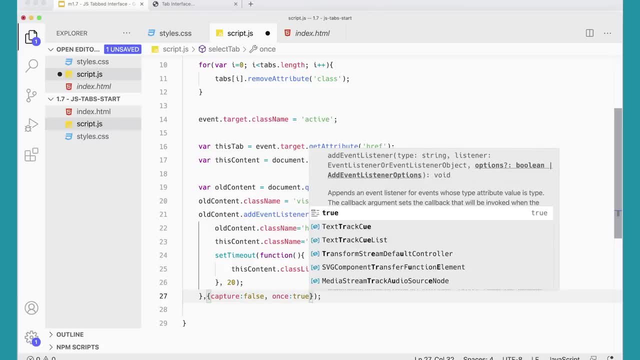 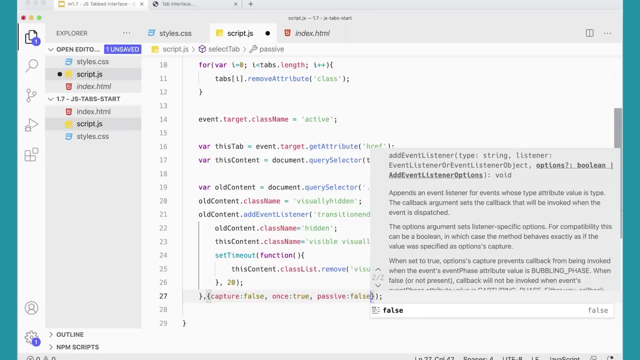 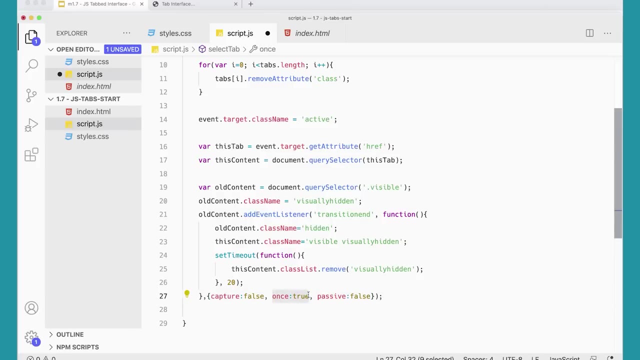 true and passive false. the only one we really care about here is this: once true. what once true does is it says: add this event listener once and then, when you're done with it, remove it, so that will get rid of that problem. capture and passive false by default. 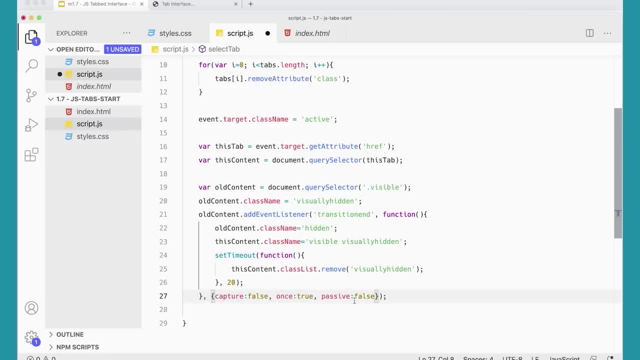 if you don't put this thing in here at all, then they're all here, but they are all false by default. so we're leaving these two as false, but we're making this one true. we have to put these two in for you to just change this one. 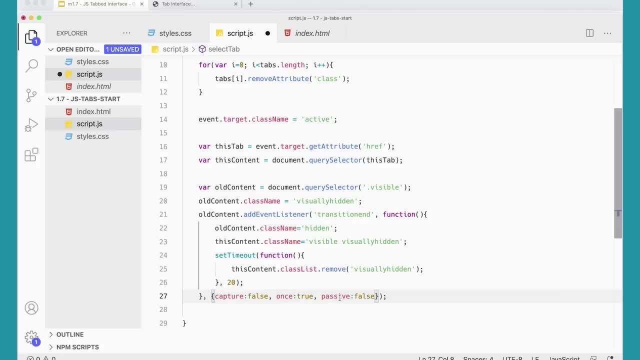 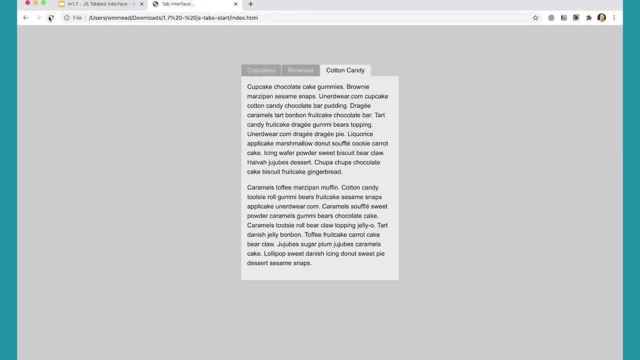 so we pass in this little object here that has capture false, once true, passive false, and if we save that and come back and refresh the page over here now, you'll notice that it will run. but it's only. it's dispensing of that event listener after the first time. 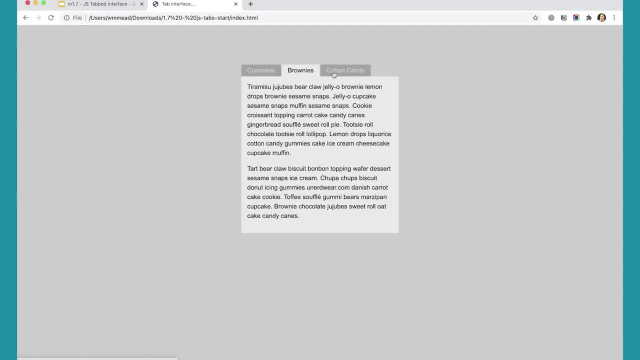 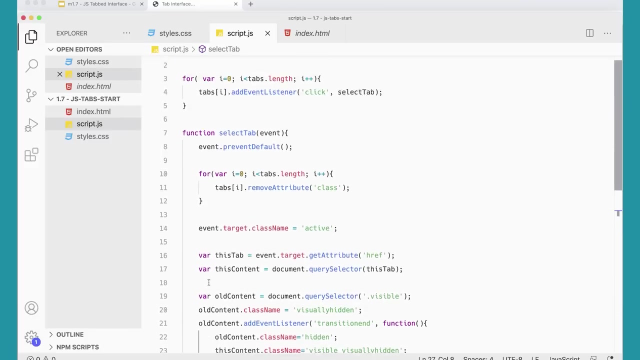 so now, when I click on it again, it's just doing it properly. it's getting rid of the old event listener and adding a new one. so that's working perfectly fine. that's great. so now at this point we have a working, functional script over here. we can. 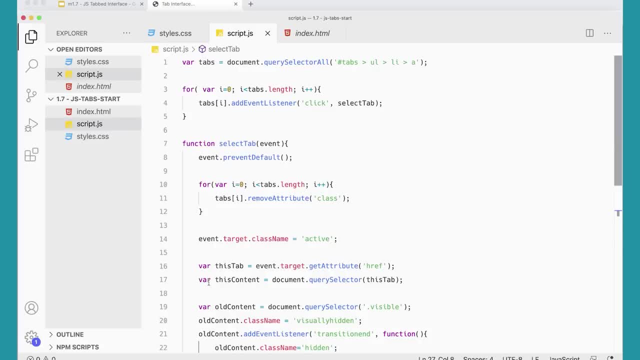 look at this script and it's a lot more complicated than the jQuery version. I think we can all agree that this script is a lot more complicated than the jQuery version and part of your decision as to which one you would want to use if you wanted to include such an interface. 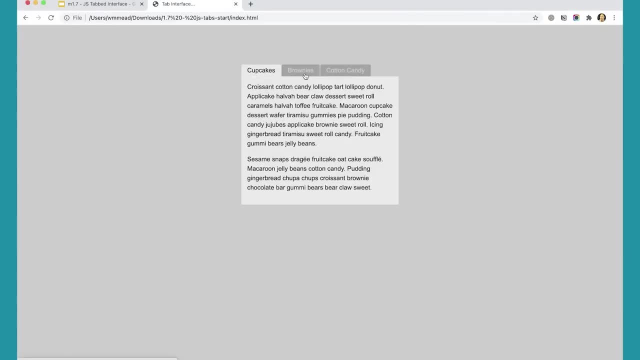 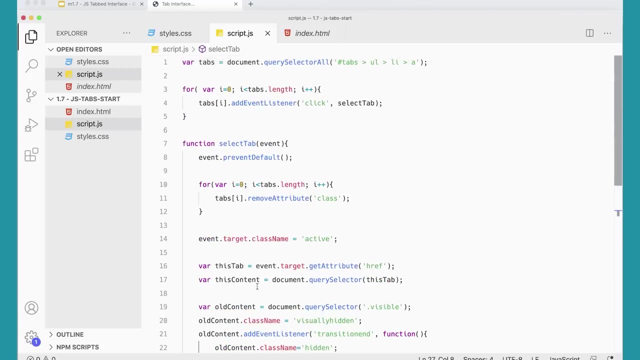 on a project of one sort or another is: is it worth including the entire jQuery library in order to have a shorter script here, or is it better to have the longer script and make use of CSS and do this kind of stuff? so we're going to do a few more things. 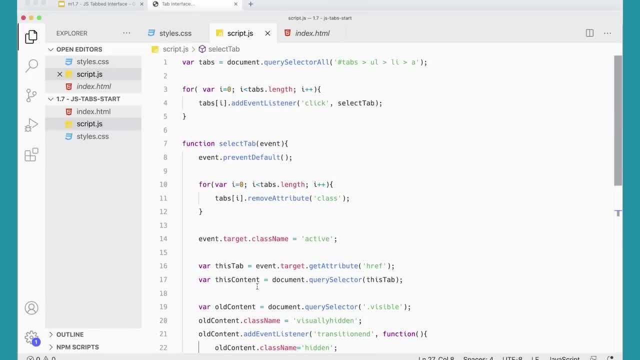 to make this a little bit better and to make it a little bit more efficient and perhaps a little bit shorter and easier to read and all of that stuff. so we're going to add those things in next. the first thing, of course, is to just do our best practices. 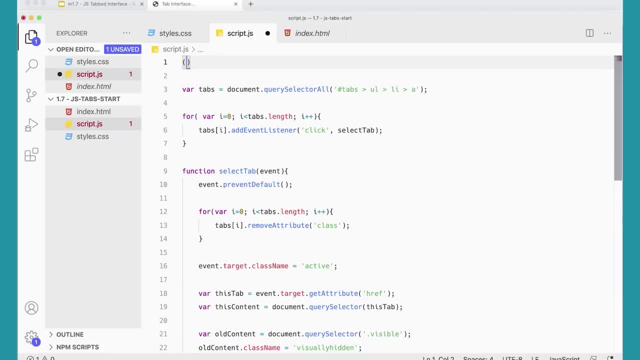 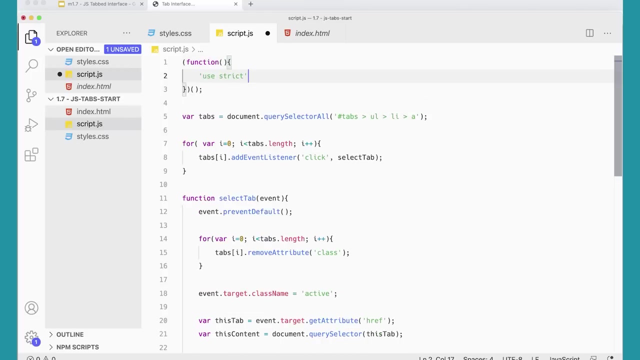 and add in here our IIFE, our immediately invoked function, expression function, parentheses, curly braces with a set of parentheses at the end and a semicolon, and then in here we can put our use strict directive like so, and then we can just make some room here and we can move this whole script. 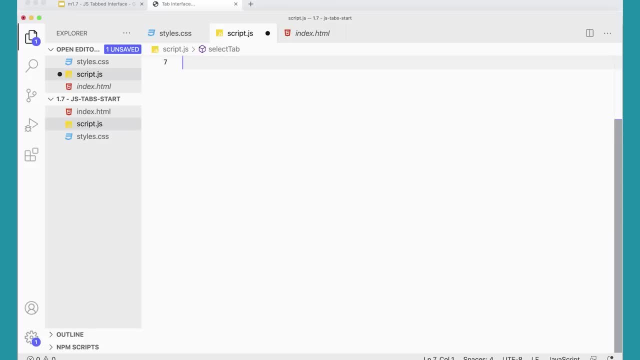 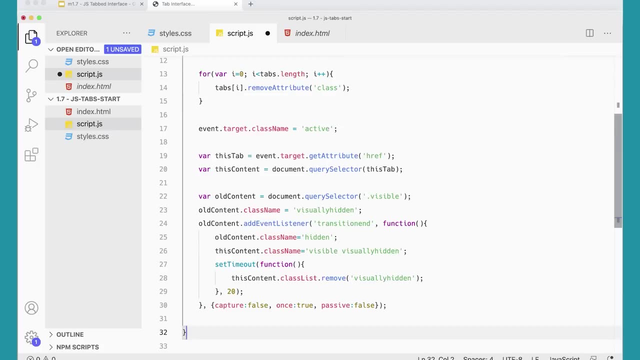 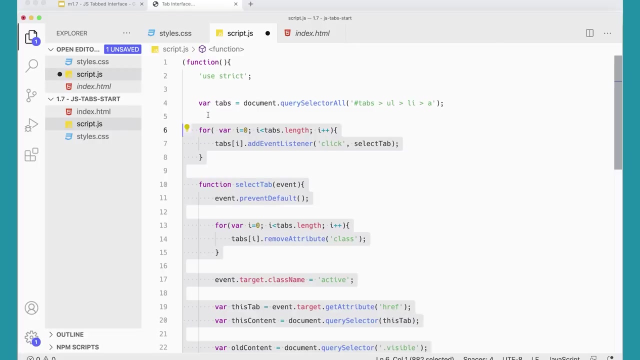 into there like that, and I'm just going to tab everything in and of course we can go through and we can change var to const. if you didn't do that right from the beginning, that can be const. this one has to be let because it's inside of the loop. 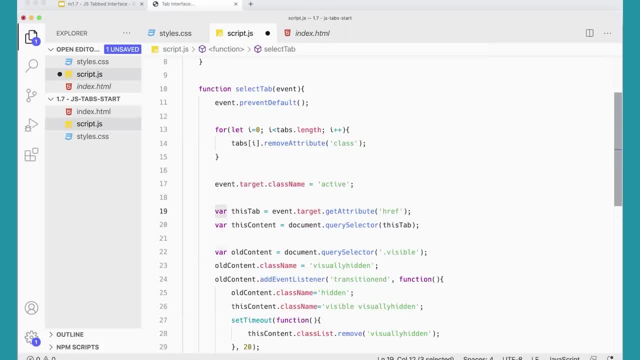 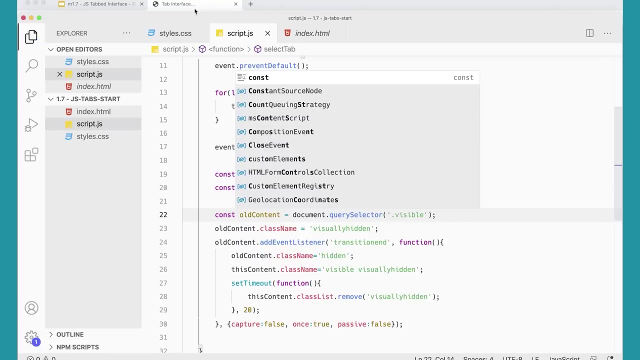 down here. this one needs to be let, and then these can be const here, that one, that one, that one can be const, and I think that's it for that stuff. so that should all work. let's just test it. make sure I didn't mess anything up there. 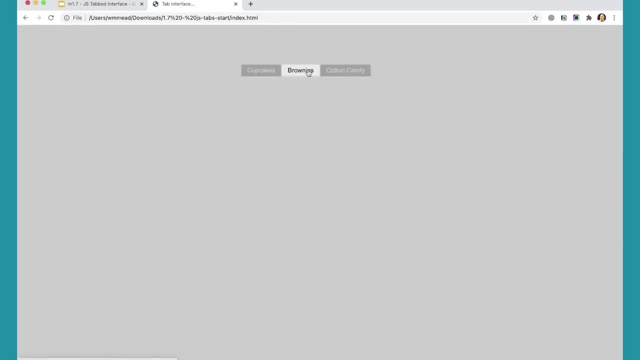 I think it'll work. yeah, that works fine. I didn't break anything, so that's cool, okay. but there are a few more things that I want to show you that we can do with this script to make it a little bit, a little bit better and a little bit more modern. 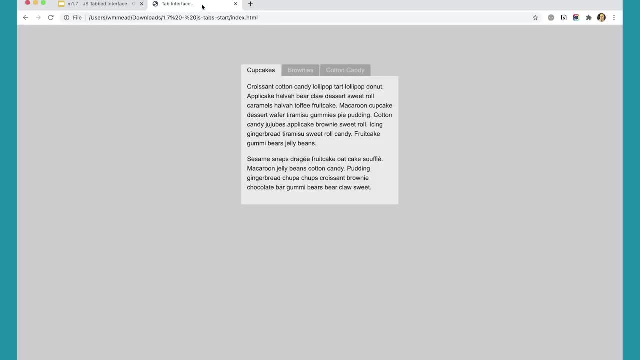 and there are things that we are going to um talk about in more detail in a later lesson, but I think it's kind of good to introduce them in these small projects so you can kind of get used to them before we talk about the theories behind them. 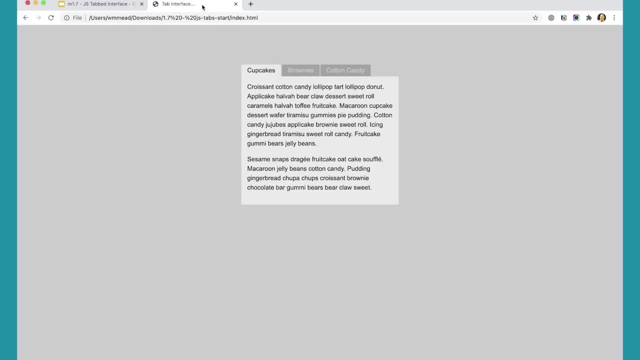 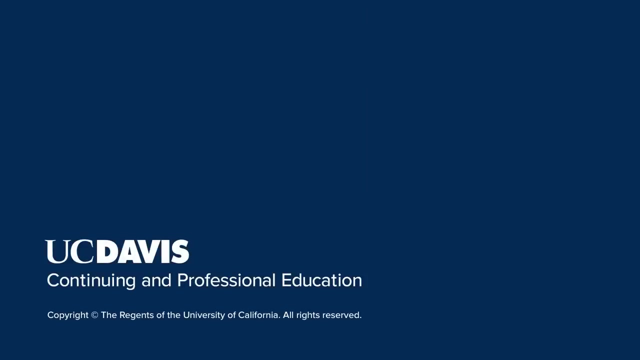 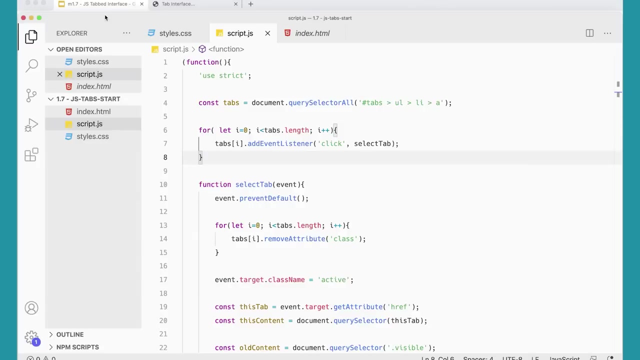 and um really delve into them in more depth. I think it's nice to sort of come into that kind of conversation with a little bit of experience with them. so we'll look at those features of JavaScript next. as mentioned in the previous video, this script is definitely longer. 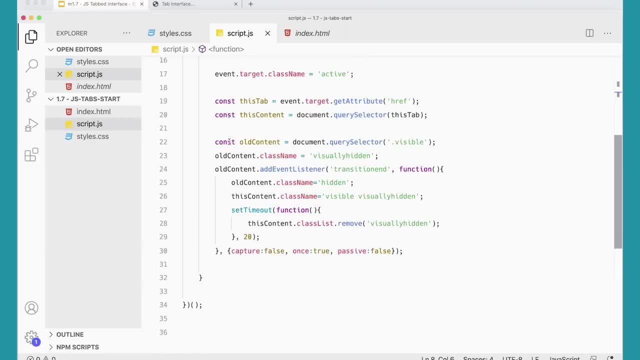 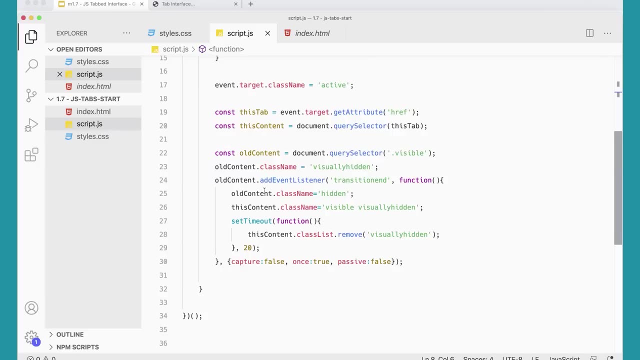 and more complex than what we would see in um, with the jQuery script, and there are some things about it that are always going to be a little bit confusing and hairy, like this transition to end thing with the capture and once and all that stuff down there, as well as using setTimeout. 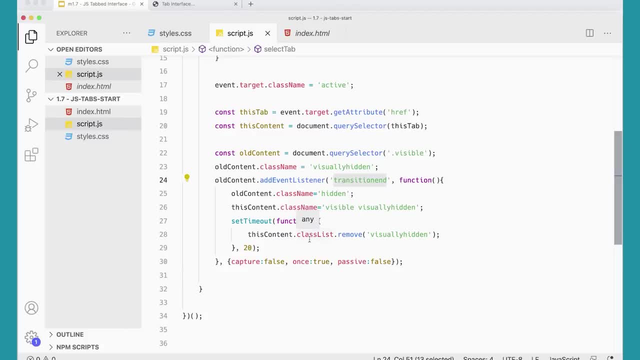 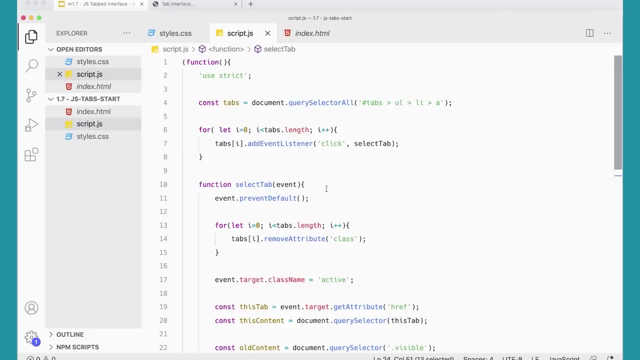 a split second before swapping the classes to get the transition to work properly. but there are a few things that we can do to clean up the code a little bit and make it a little bit better. and again, you don't have to do any of this. you can leave the script the way it is. 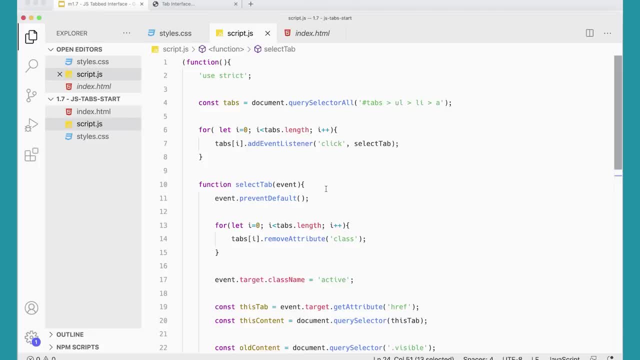 it works fine the way it is. these are just some things that are worth looking at and thinking about in terms of syntax for JavaScript, and we'll get into these features in more depth later. this is just a good opportunity to introduce them. one of them is the forEach. 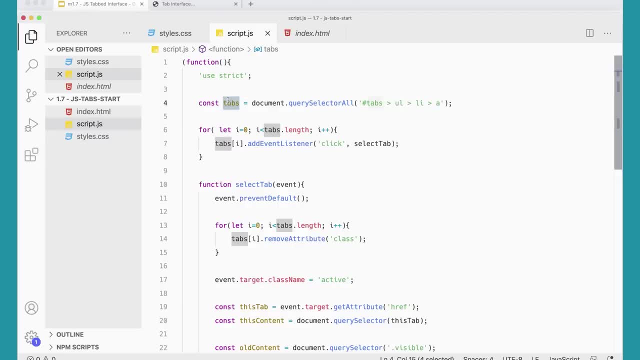 method which can work on arrays. tabs is an array because it's going in and getting all of the all of these tabs and there's just three of them. but it's an array and the for loop is fine. it works fine, but it's a little bit hard. 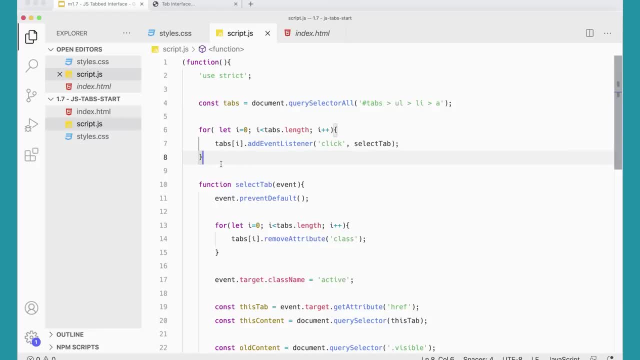 to read and a little bit cumbersome, and the forEach method is a little bit nicer, so let's just try that and see how that looks instead. so what we would do is we would say tabsforEach, like this: this is the forEach method, and the forEach method- again, it's an array method, so it works on arrays. 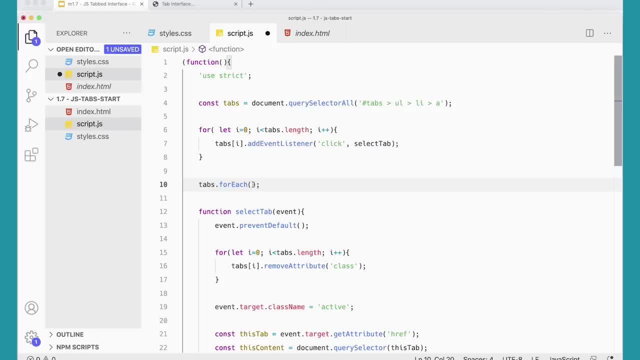 so we do tabsforEach and we pass in a callback function that runs and this function takes a variable that's going to work on each element in tabs and you could call it each tab or you could call it tab. so it's going to do something with tab. 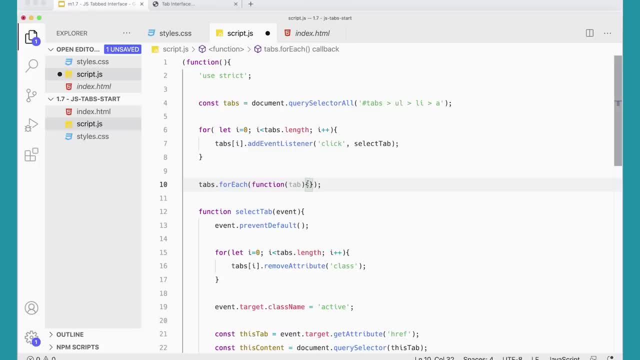 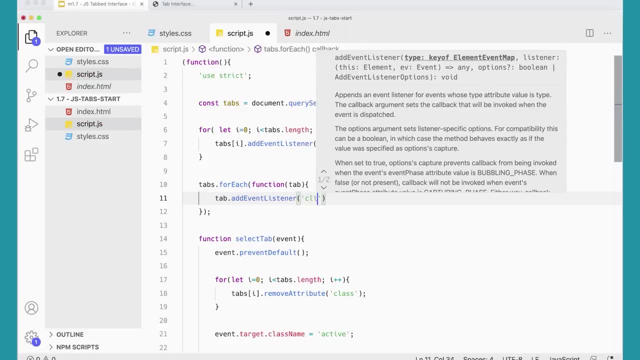 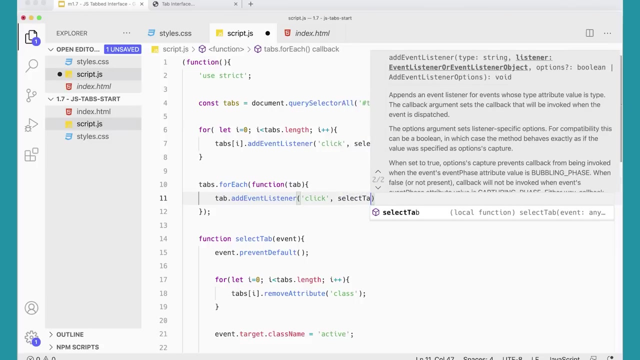 so it's going to go through each of the tabs and do something with tab, and what are we going to do here? we're going to say tabaddEventListener and we're going to do click and then we're going to run this select tab down here. so this 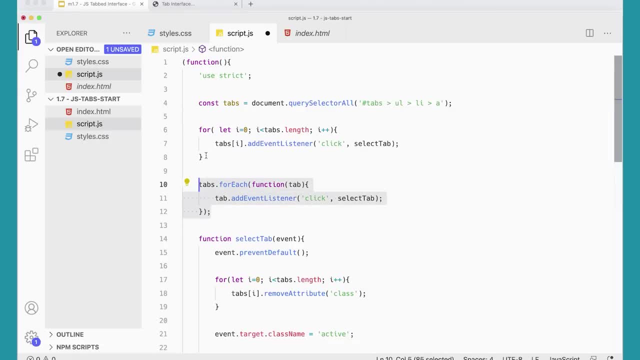 piece of code is doing exactly the same things as forEach here, so you could either comment this out or delete it all together and just use the forEach method here. that will allow us to add an event listener to each tab, and I just think it's a little bit. 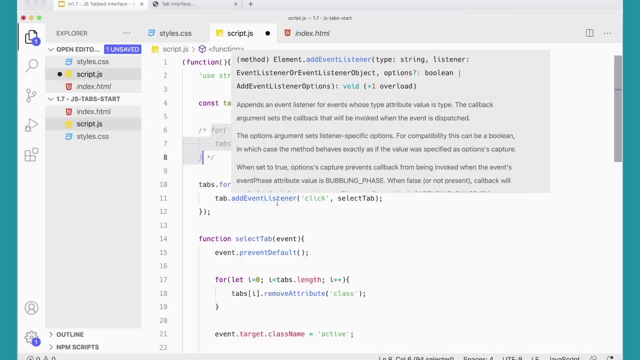 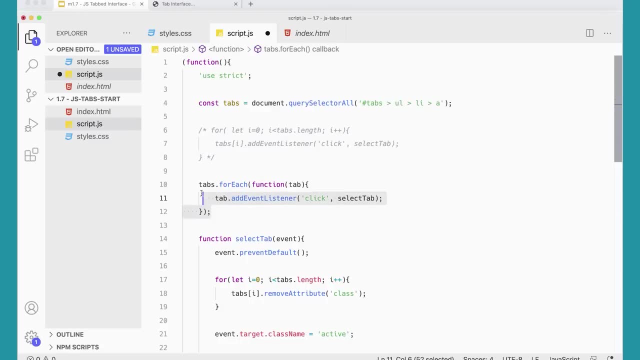 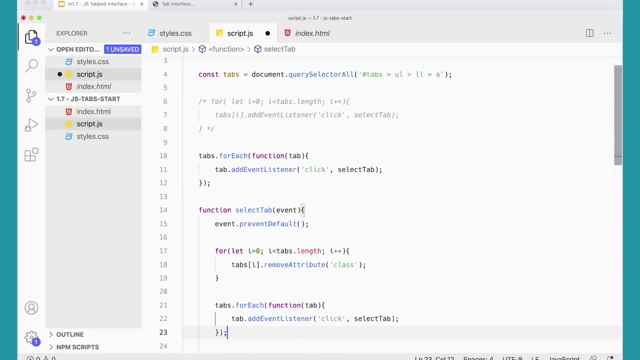 easier to read- and again, we'll get into this more later- but this is a good place to introduce it, and we could do the same thing down here in place of this forEach down here as well. we could even just paste this in, but instead of adding an event listener. 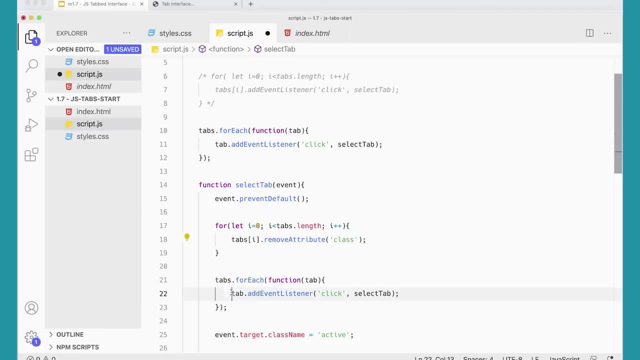 we can just do this instead. but instead of tabs dash square bracket i, it's just tab remove attribute class. so again, we're just replacing this for loop with that, and that should work just as well as before. so let's go over and just test this really carefully here. 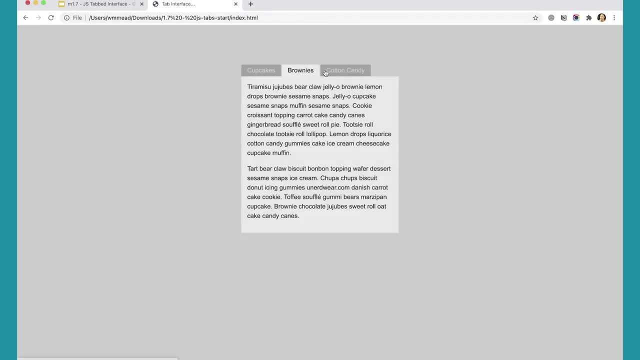 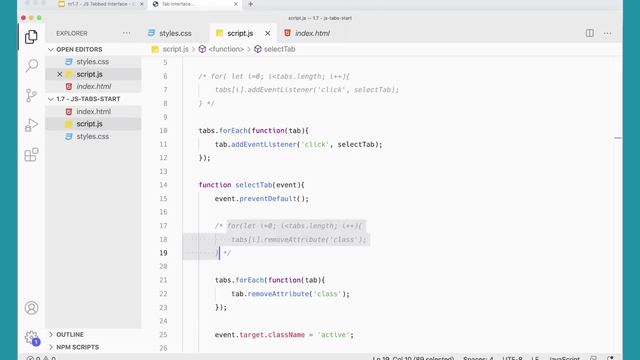 so if I refresh this and test it, you can see that it's working exactly the same as it did before and and that's great. so you can get rid of these things here now. even further in in javascript, there is now a something called an arrow function, and if you've looked, 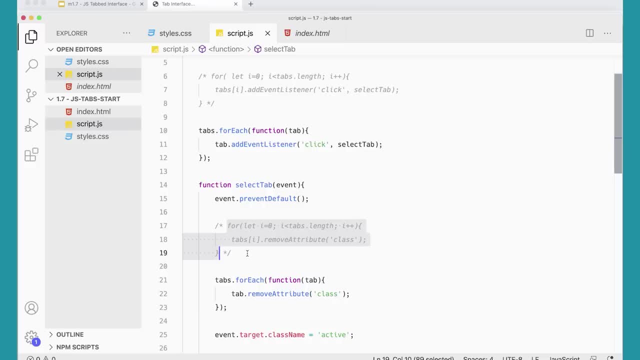 up javascript online. you've probably come across arrow functions before and again, we're going to get more into arrow functions and sort of talk about them in more in depth in a future lesson. but this is a good place to kind of introduce them, because we could even 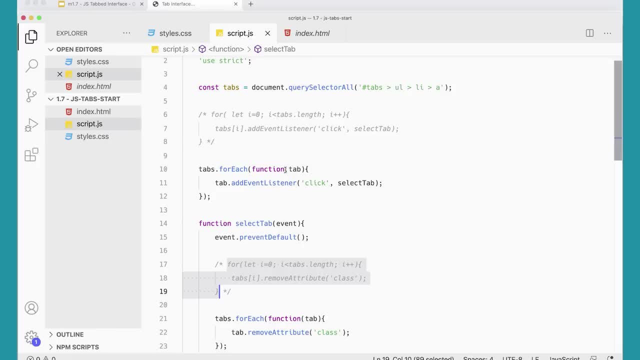 further clarify these little functions here with arrow functions, and the way they work is like this: you get rid of the word function and instead over here you put what they call an arrow, which is really just an equal sign and a greater than sign in here, and if you're 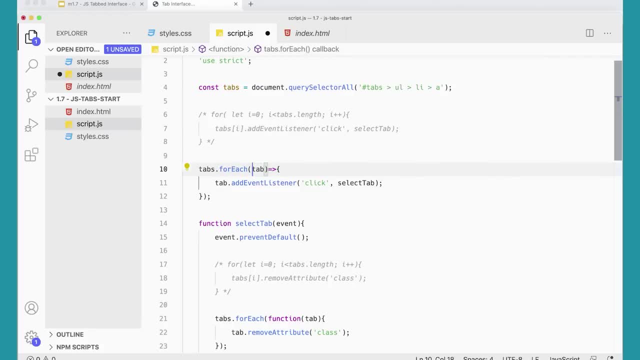 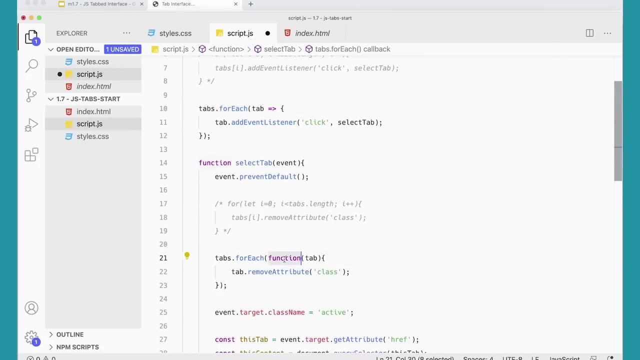 passing in only one variable, you can get rid of the parentheses. so now we have tab for each tab and then this becomes the function that runs, and we could do the same thing down here and again. we're going to do this in more depth later to talk about. 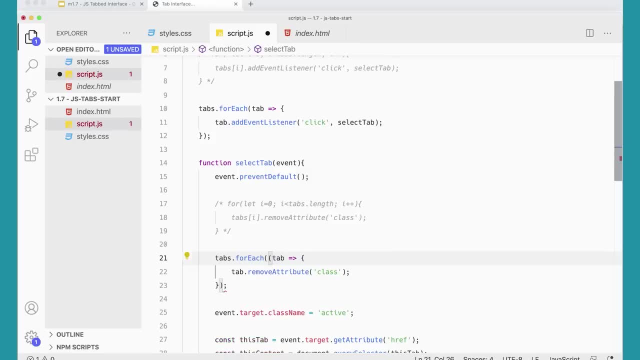 arrow functions and when to use them and when not to use them and what they're good for. but this is a good place for them and it just gives us kind of a really clear tabs for each tab. we're going to do this kind of thing. you can even move this up, so it's all. 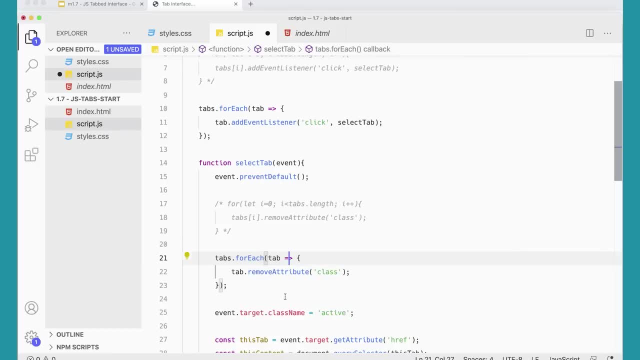 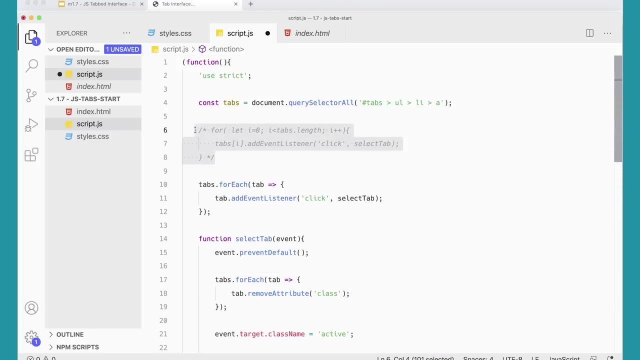 in one line practically, and so it becomes so short and clear and that kind of really helps with sort of the clarity of the script. I'm going to get rid of this, just to make it a little bit shorter. um, leave that space there, and up here I'll do this. 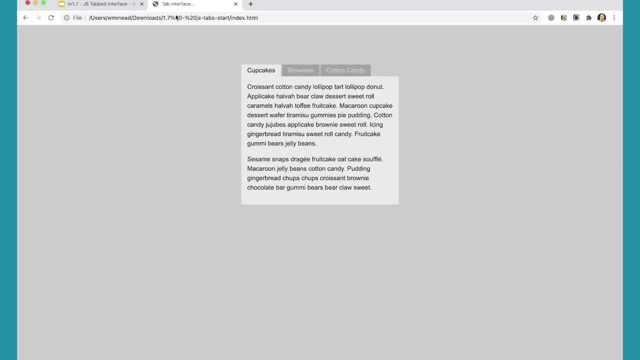 and it should work just the same as it did before and again. you don't have to do any of this stuff if you don't want to. the script worked perfectly fine before and there's nothing wrong with using the for loop and not using the for each. 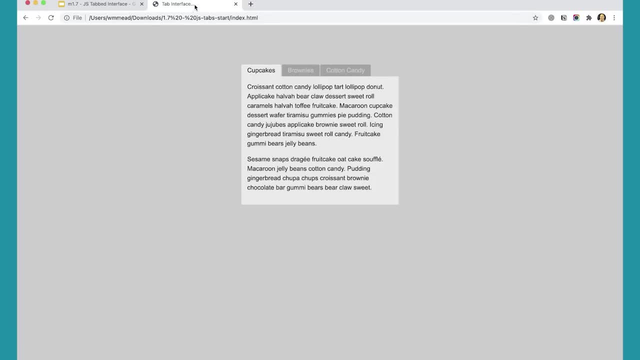 or using the arrow functions, but it just seemed like this would be a good place to introduce those ideas and just to summarize up the lesson, what we've done here is we've taken, we've created a typical interface element, a tabbed interface, and we've done it. 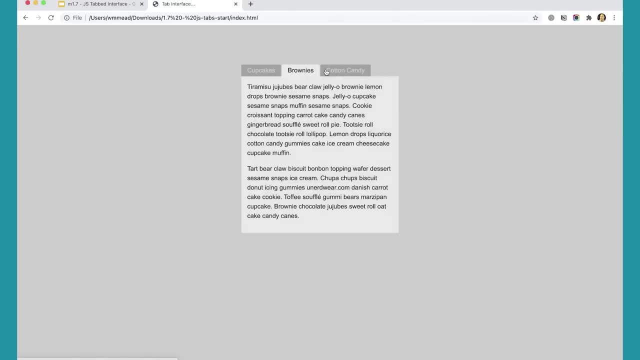 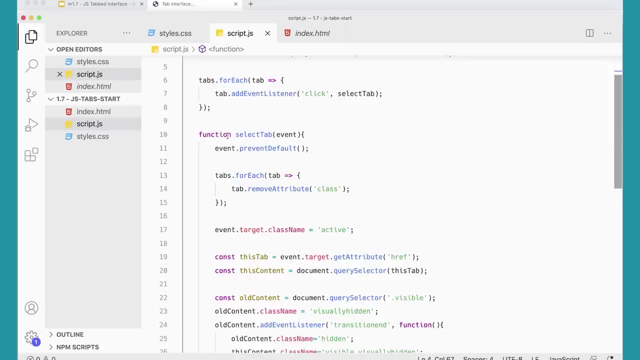 with plain javascript and it's a little bit different than the version that we did in jquery and ultimately you have to decide whether including the jquery library and doing the shorter script is worth it for making this thing. and it's not that long, it's not that bad. 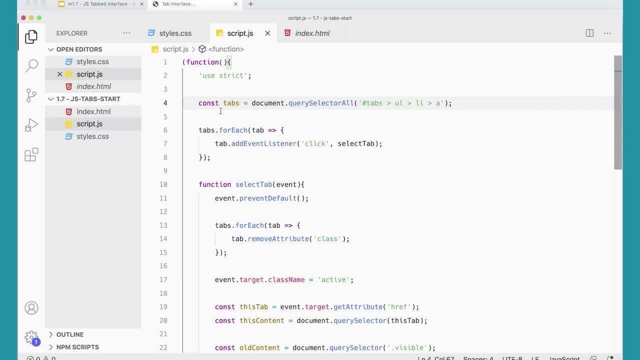 and it's certainly a lot less code to download than the entire jquery library. on the other hand, if you're using jquery for other things in your project already, then you know using it for the tabs doesn't actually add any extra weight and it works really well and it's short. 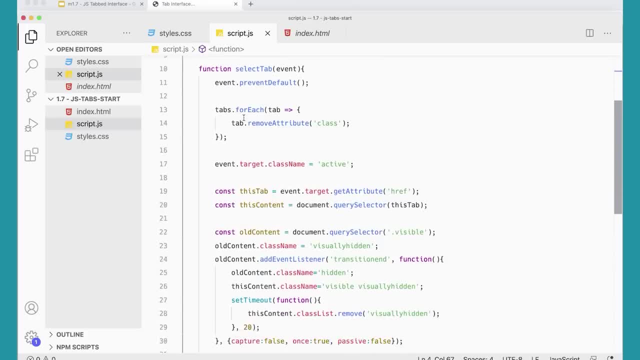 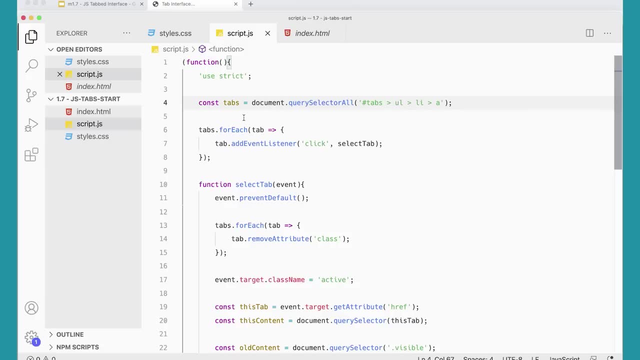 and quick and right to the point. so this is a really great example of the difference between javascript and jquery. and again, jquery is just more javascript, but but there are differences with the way the syntax works and you can write shorter, more efficient scripts with jquery, if that helps you. 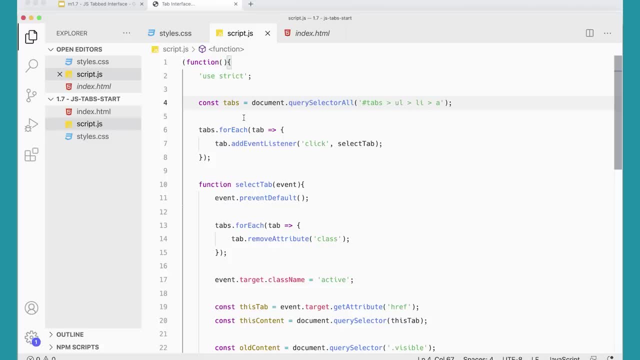 get used to working with javascript and more excited about learning it, then by all means use the jquery. if you prefer to really learn the plain, vanilla javascript because jquery is starting to get phased out- then this is a really good example of the kind of work you're in for with plain javascript. 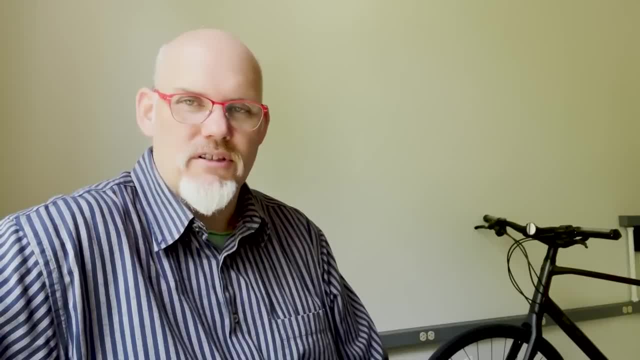 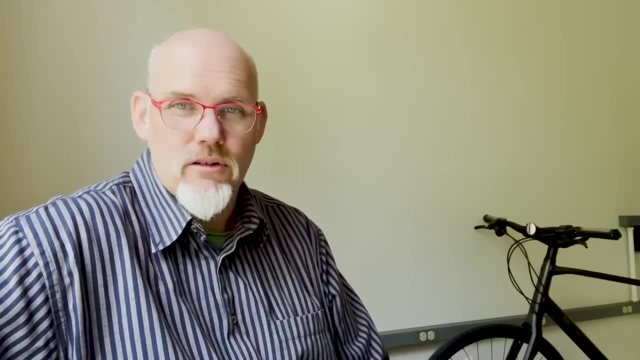 welcome to the third module in our second course on javascript. in this module you'll create some scripts that are useful and that you can put on actual web pages. plus, they'll build your skills and you'll get better at working with javascript and jquery. they provide a 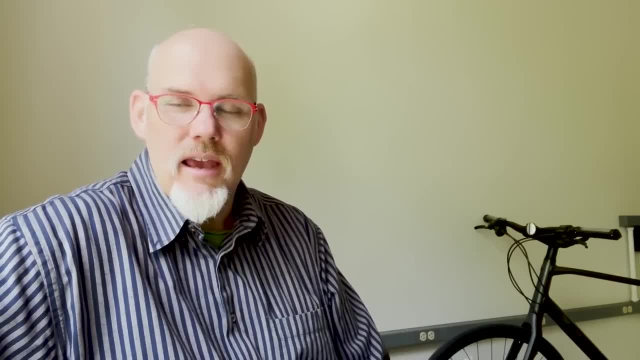 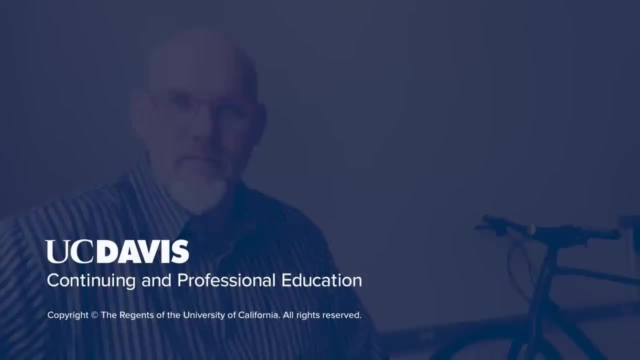 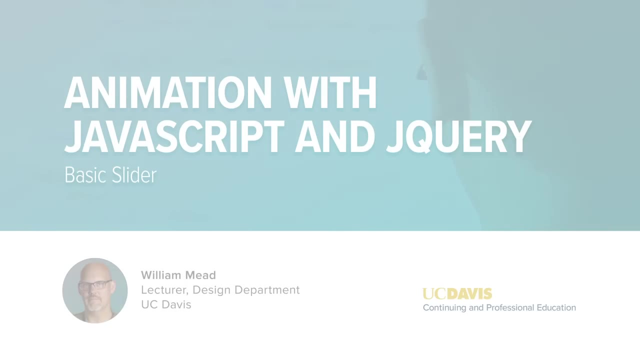 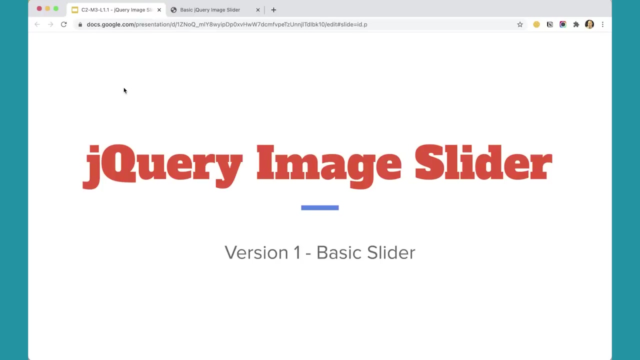 lot of practice, so let's dive in and start working on these scripts. i think you're going to get a lot out of them and i look forward to going through them with you. jquery image slider- version 1- the basic slider. learning javascript and learning jquery is most fun when you're actually working. 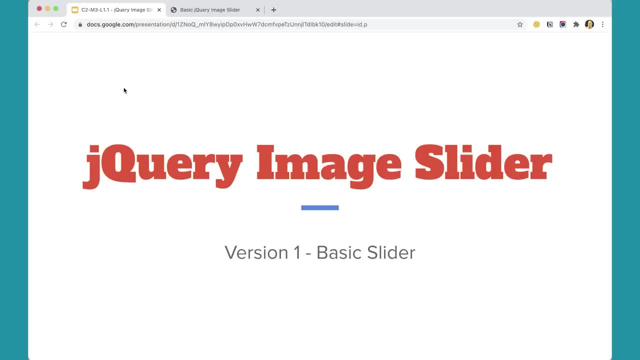 on projects that you could actually use, and in this lesson we're going to make a basic image slider that you could put on any website, and that's pretty exciting and pretty awesome to be able to make something you can actually use. plus, along the way, you'll learn some new. 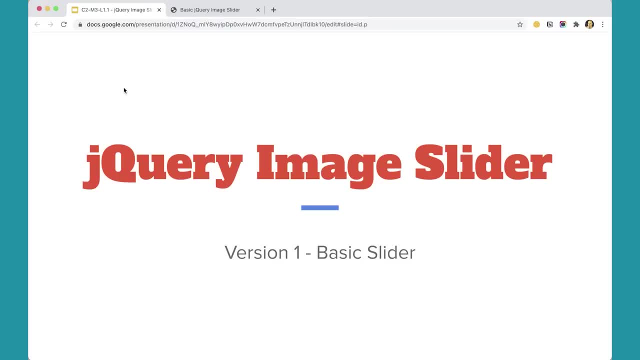 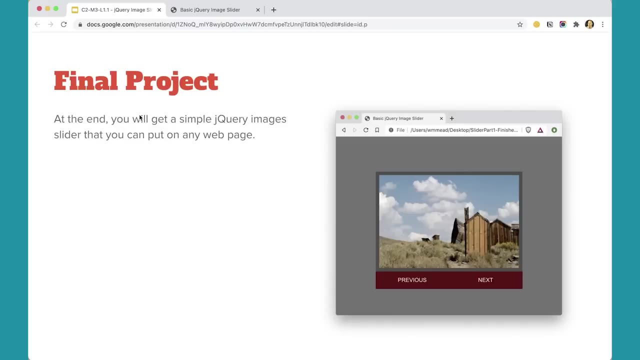 things about jquery and some new things about javascript and get a lot of practice and and really this is a great way to learn javascript and jquery. so let's move forward and see how this project works here. the final project, you'll have a just a simple little uh slideshow that 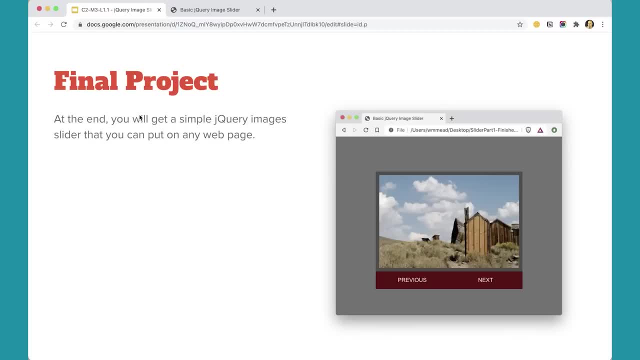 where the images will slide from left to right, or they'll come in from the right hand side and slide over to the left hand side as you go to the next image, and then the other way around as you go to the previous image, and we'll see how that actually works and how it comes out as we move. 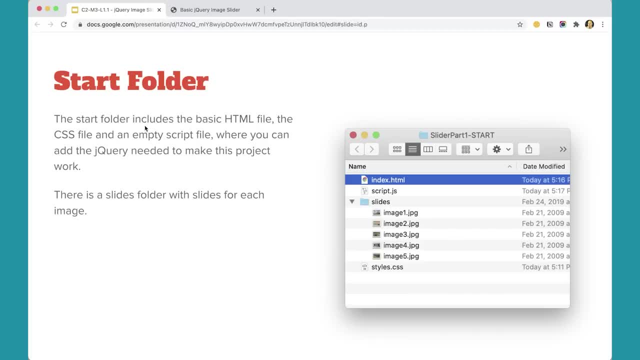 along here in the start folder. so download the files to go with this assignment. in the start folder you'll find there's an index HTML file, we've got a script file and we've got a folder with some slides, with some images that I took up at Bodie National Park, which is a an old, abandoned ghost town, and it's 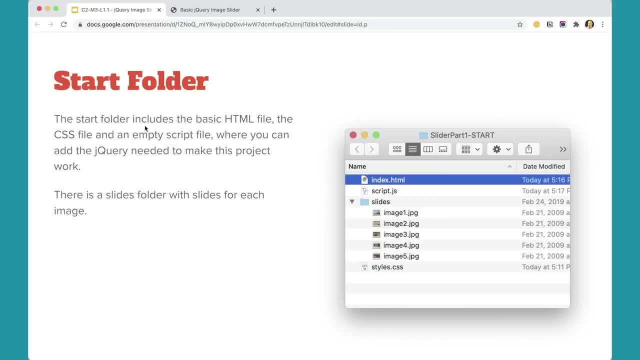 pretty. it's a pretty interesting place. lots of great places doing great place to take a lot of great photos. so I took a took some photos up there, so we'll use some of those for this project and that's kind of fun and if we come over, 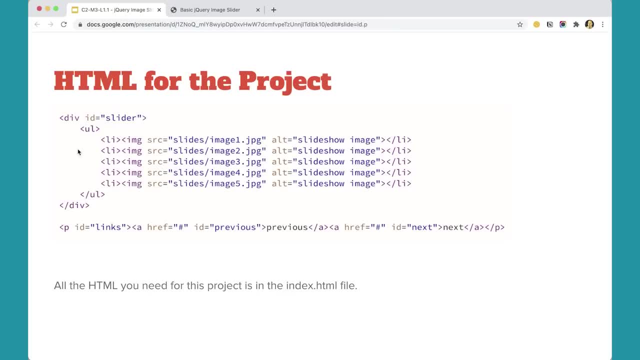 and look at the index file, you'll notice that we have a div with an ID of slider and then an unordered list with list images, list items for each of the images, for the slides in the slideshow, and this is actually a fairly common set of slides that I've used for this project and I've used it for a lot of. 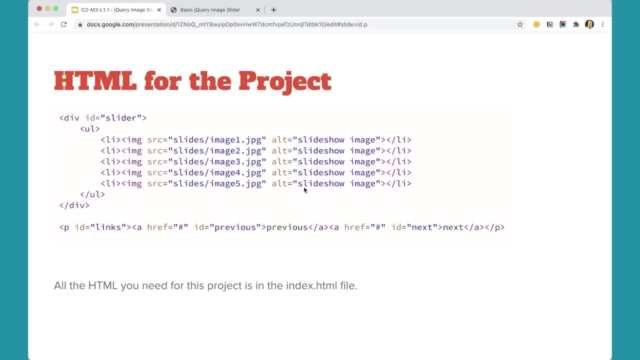 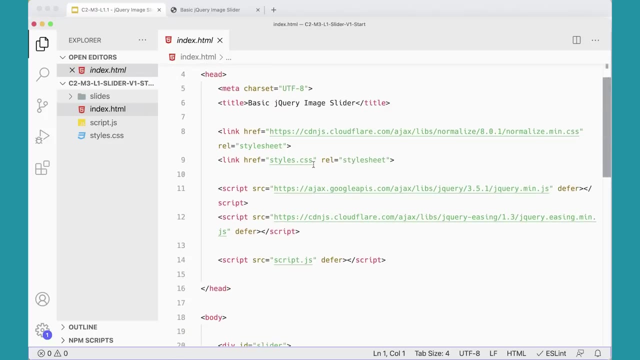 other projects. but I'm actually going to show you guys a setup that you'll find for image slider scripts that you might find around the web, and then I've just got some links for the previous and next buttons. so if we come over here and actually look at that HTML, you'll see that that's what it looks like here. I'm 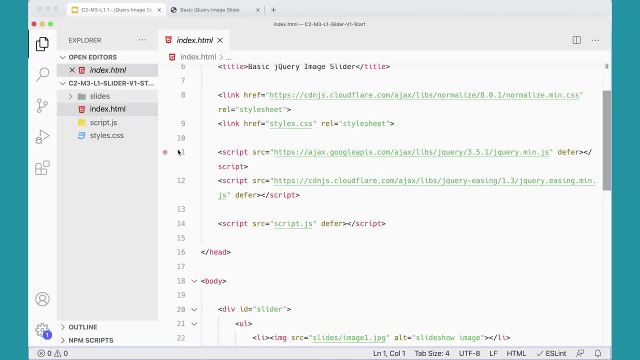 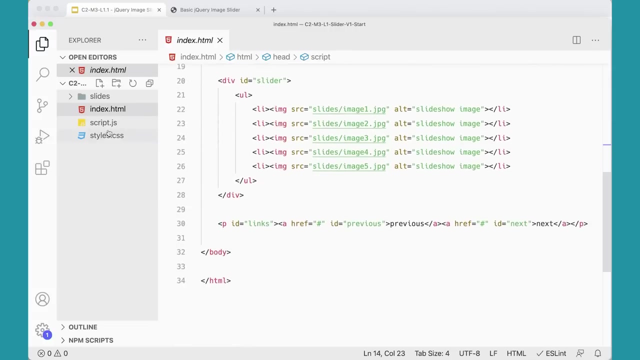 loading my normalize script. I've got my CSS, I've got jQuery loaded here. I'm loading an easing plug-in that we'll talk about in a bit- and then we've got our script file here and then we've got our slides. so that's all there. 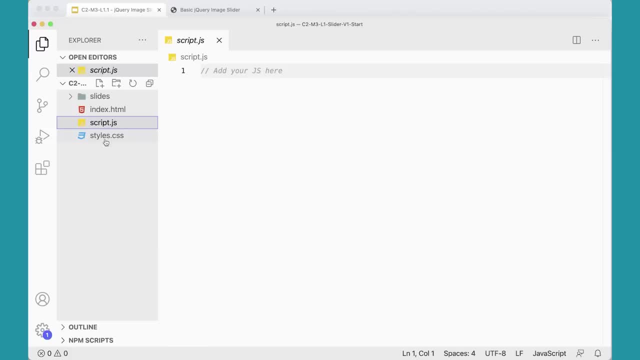 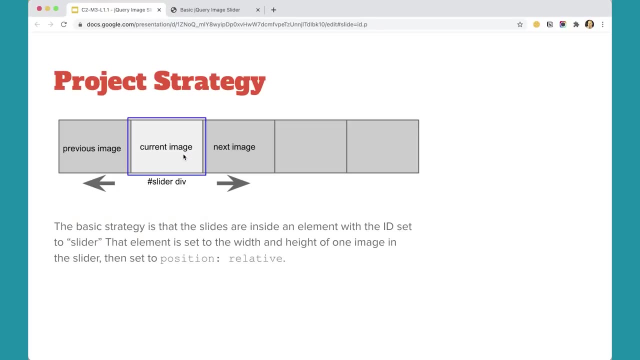 I've got a script file here which is empty. that's, we're gonna write our JavaScript, and then we've got some styles that we'll talk about in just a minute here. the important way to think about this- is the important strategy here- is that the images are all going to be lined up in a row, and what we have as 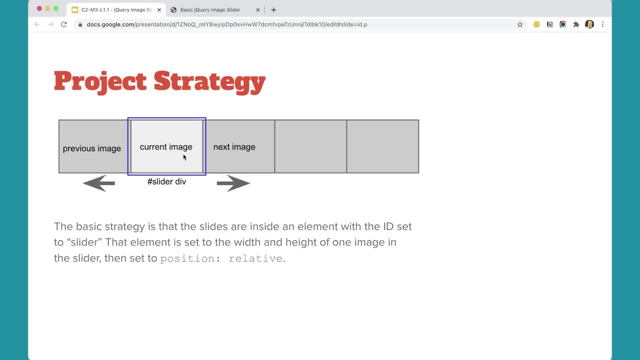 the actual window. this slider div is gonna have overflow hidden on it so that you can't see the other images, and it's gonna be set to position relative so that we can absolutely position the string of images, the strip of images, inside that window. so the current image will be displaying and when you click, 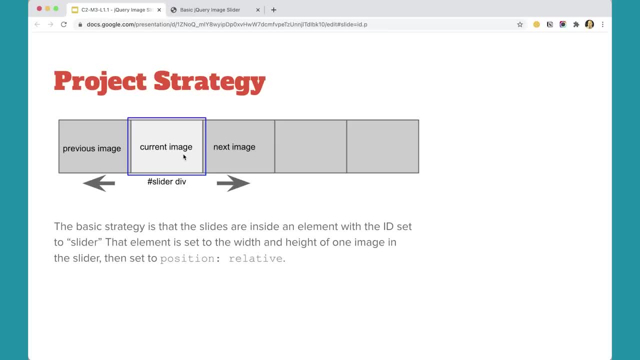 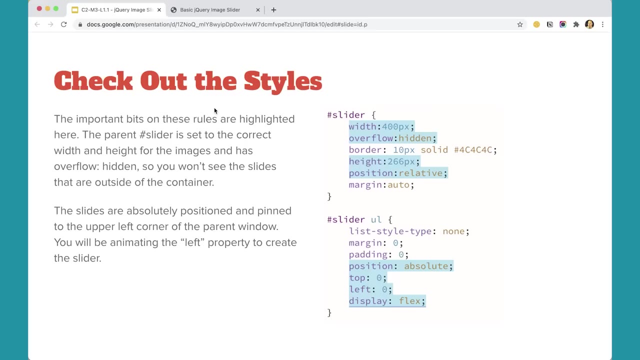 next, the next image will slide in, or, if you click previous, the previous image will slide in, and that strip will basically slide back and forth left and right as we move through the slides. now one thing to check out is the way that the styling works, and it's really important to understand the way HTML and CSS works. 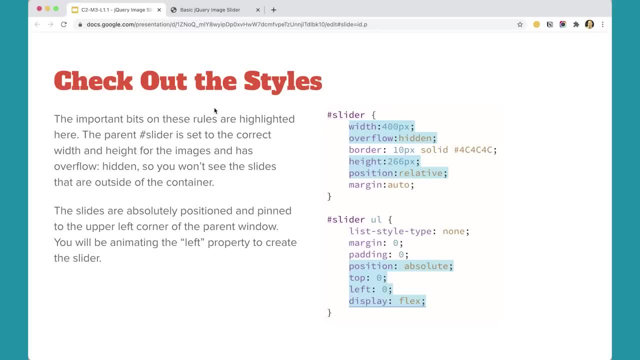 because it's these tools that will provide the basic content and structure for our pages and even though we're learning JavaScript and that has to do with the behavior, the behavior very much is affected by the layout and content of the pages. so we're going to take a look at that and we're going to go ahead and 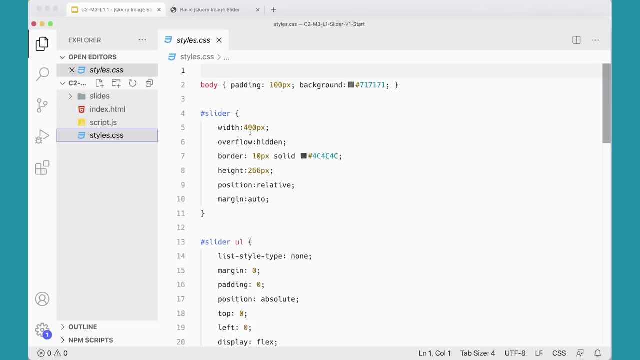 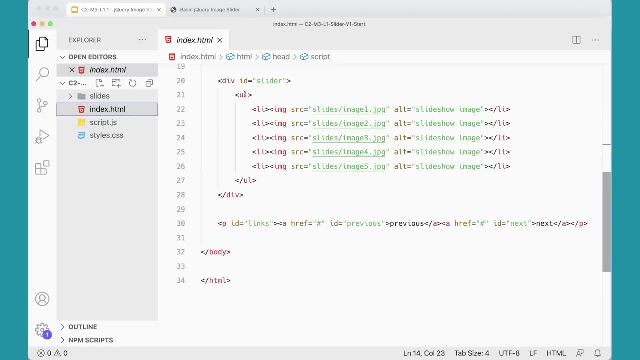 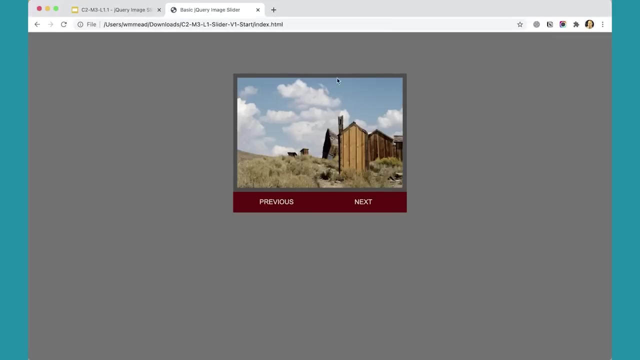 and look for something in the menu. so ifwe come over here and look at this, the overflow hidden on this slider element here, which is again if we go back to the index here, it's this div here. if I come and look at the page, it's this div here in this div here that 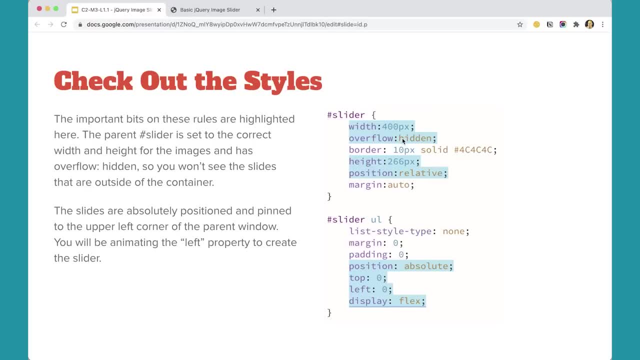 has the picture in it and that div has overflow hidden on it and it is showing only over, over, over and over the uh the slide that is in the window and the width of it is set to the same width as the actual. 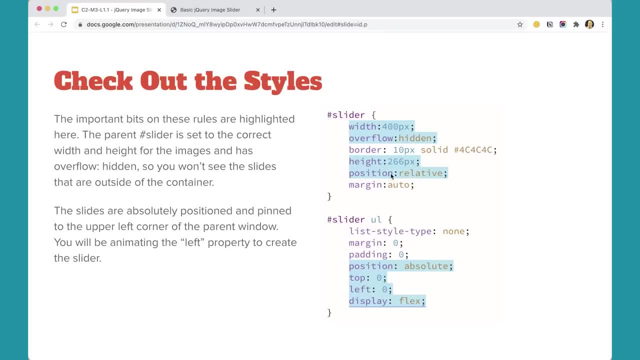 images and the height is set to the same height and then it's set to position relative. so we can use absolute positioning. and if you know some css and you know about positioning, you know that when you set a parent to relative positioning then the child set to absolute positioning. 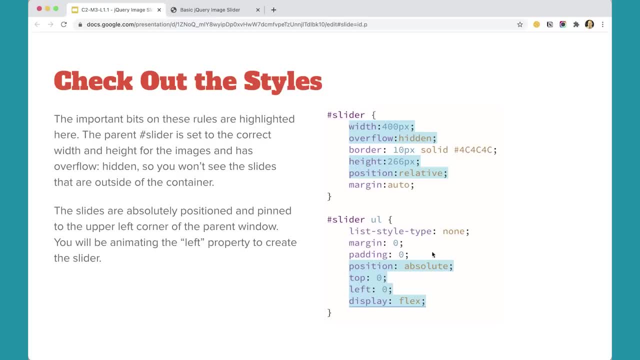 is going to be set in relation to that parent element. so position zero: top zero, left zero puts that thing in inside this container here, and then display flex is what makes all the images go into a row. top zero, left zero puts that in the top left corner. now, if i were to go in, 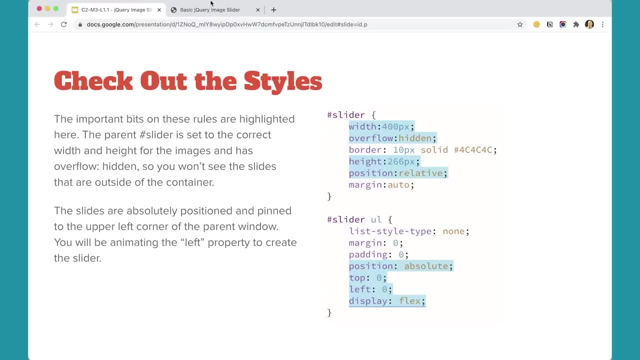 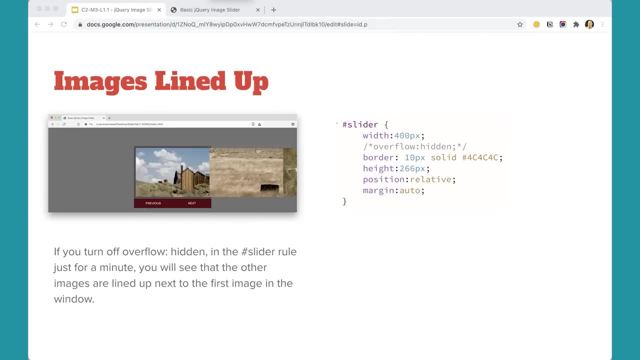 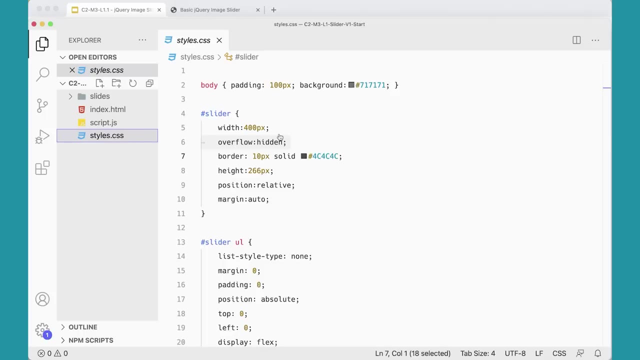 and mess with this just a little bit, you could see what it will do, for example, if i take overflow hidden out of my slider declaration here. let's do this just to see what happens if i come over here to my styles and remove overflow hidden, which is temporarily. 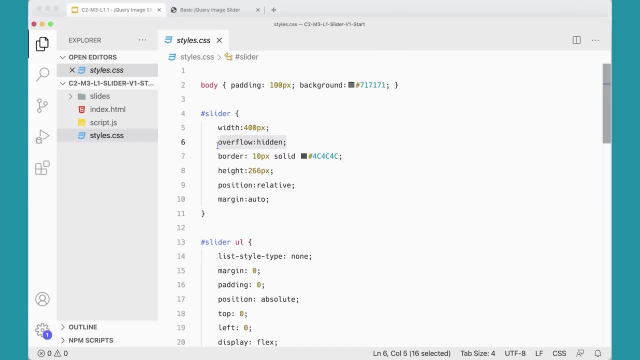 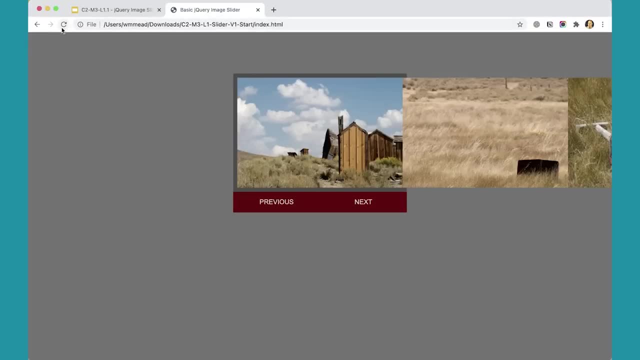 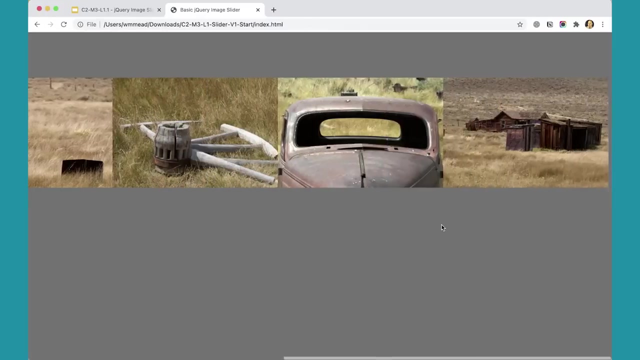 i'm going to just comment this out like so and save this, and then when i come back and actually and refresh this, you'll see that the other slides are all lined up. each one is on their next page, full音 to each other, and they're all lined up here. they're all in a row, just lined up waiting. 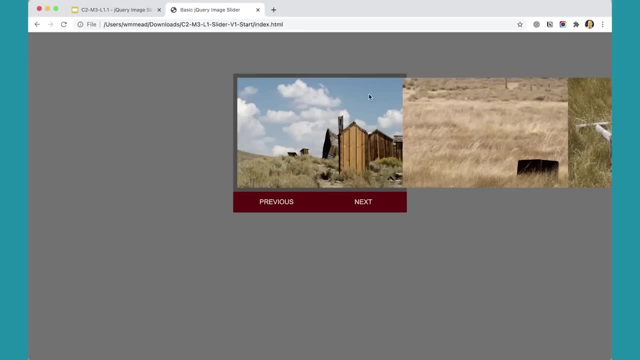 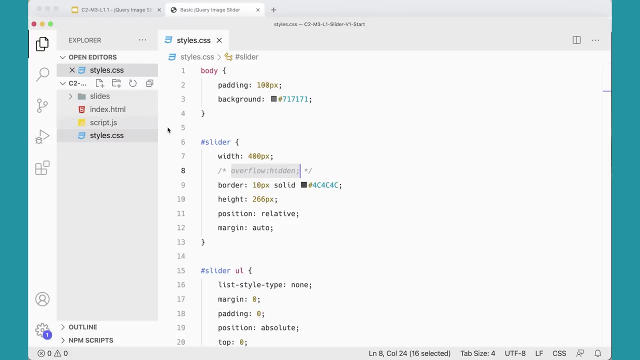 just because of overflow hidden, we're not seeing them. we're only seeing what's actually in the window. so we want to go back and put overflow hidden back. so we're not seeing those additional slides, we're only seeing one. that's actually in the window and it's important to understand that. 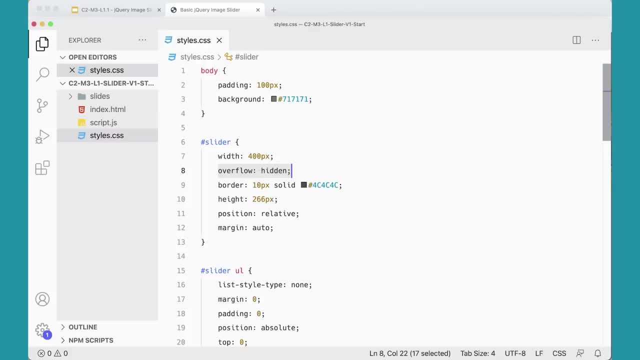 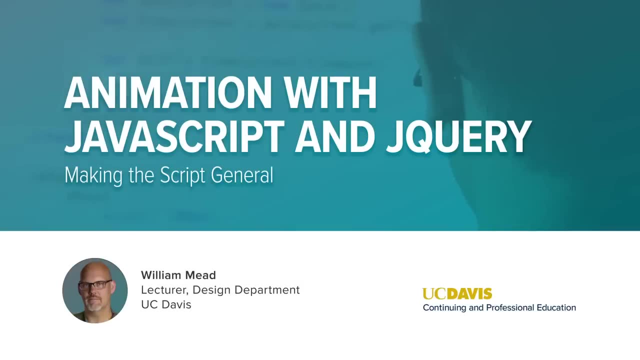 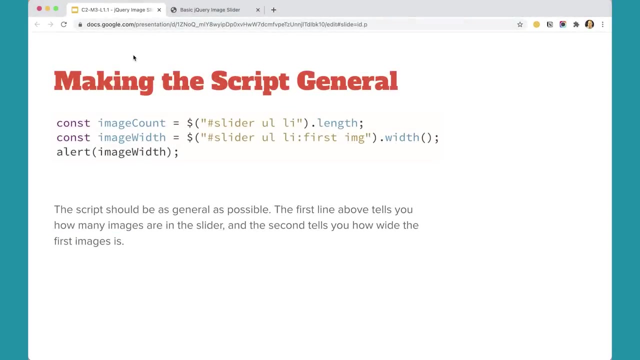 that's how this project is set up, because it has an effect on how we write our javascript. one thing we want to do as we're working on our scripts is we want to make them as general as possible, so that if we were to add more images into our slider, then our script would be able. 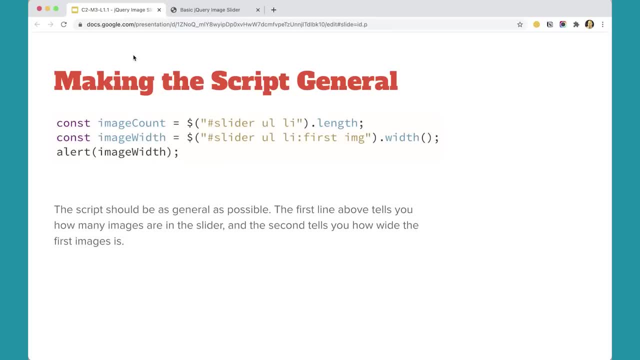 to handle them. so i'm going to use some variables to keep track of some things like: well, how many images do i actually have in my slider? i know right now that it's five and i could just leave it at that for image count. but i could just set image count to five. but 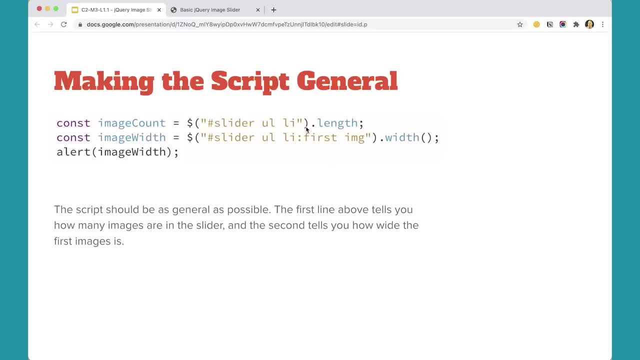 i'd really rather have it actually find out what is the length of my element here. and then i also want to find out how wide is my image, and i'm going to assume that all my images are the same width, because the slider won't look right if they're not anyway, so i'm going to assume. 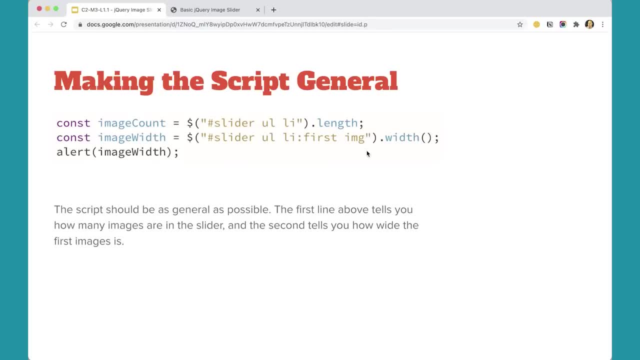 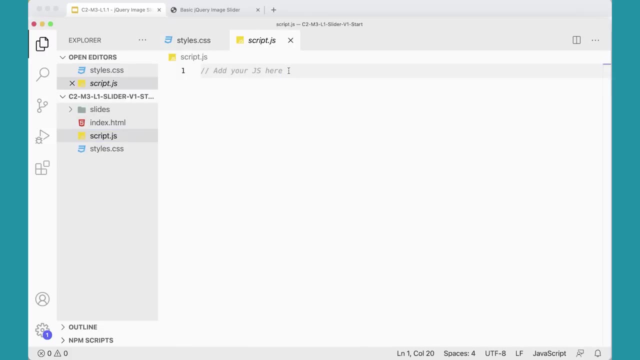 that all the images are the same width, but i need to find out how wide is one of them, and so let's go ahead and add these two variables to our script over here. so i'm going to come back to visual studio code and go to my script file, and here i can just add in const: and uh, what did i set this? 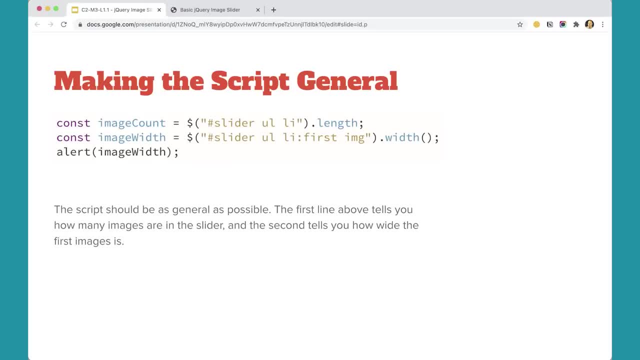 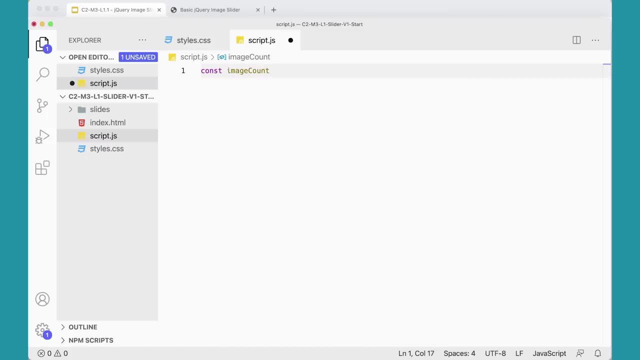 for i set this variable to image count. how many images do i have? so i'm going to set image count variable. image count. i'm going to make it equal to. i'm going to use my jquery object to go in and find out how long my- uh, my- script is. so it's pound slider ul li dot length. 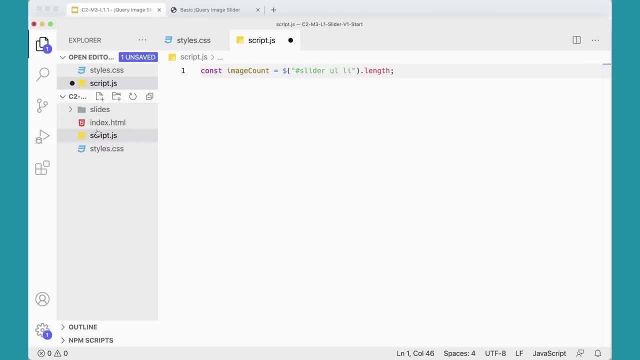 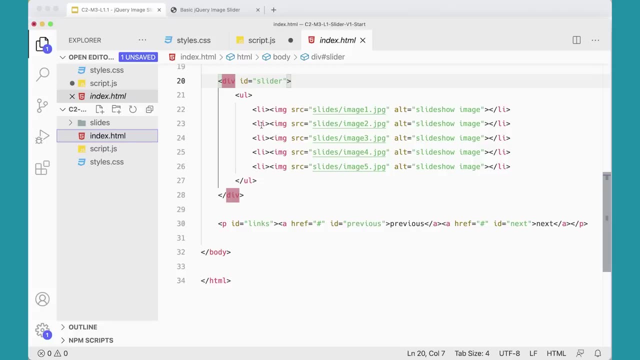 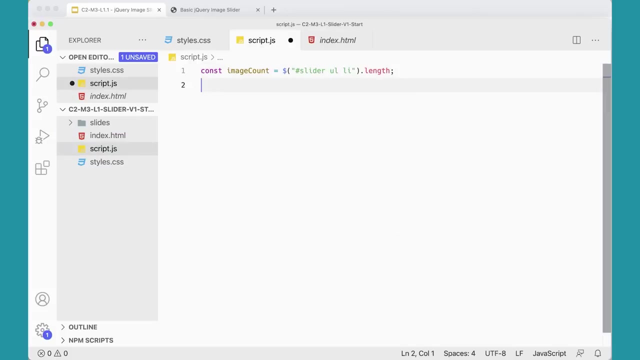 and that will actually go in to my document over here and look for this slider element and then go and find the, the list items. i'm going to find out how many are there. so that should return to me a five. it should give me five there and then i'm going to have a variable const. 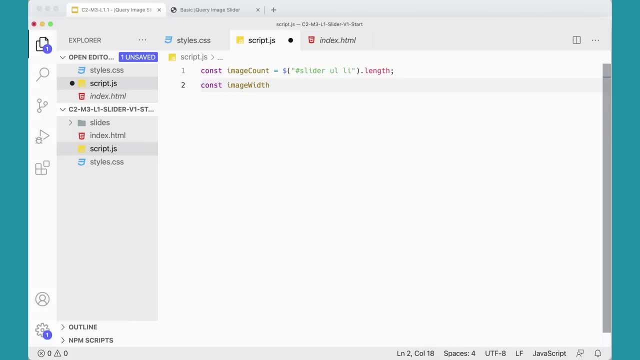 image width and i'm going to use my jquery object for that. i'm going to put in here: pound slider, ul li colon first img dot width and that should give me a number that tells me how wide my first image is. let's see what that does. alert. 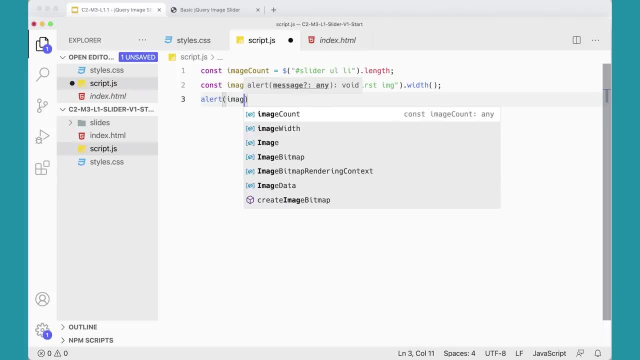 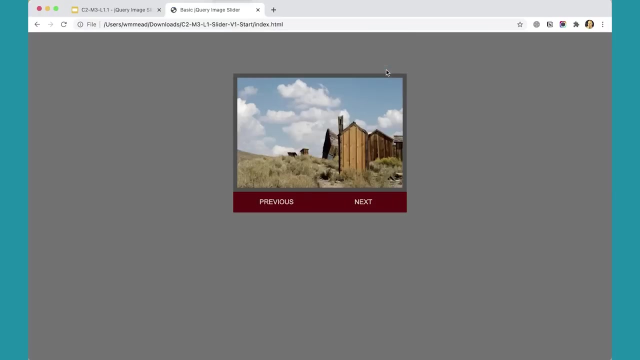 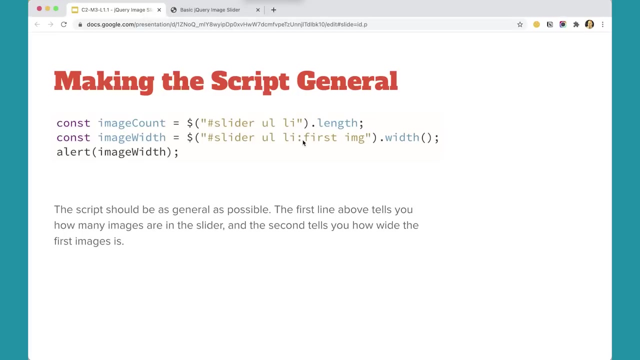 image width. save that, come back here and refresh the page and i'm getting 400.. it's telling me that it's 400 pixels wide. now, before i move on, i'm looking at my slide here and realize i'm using the this here to get the first list item. So what that does is it goes into the DOM here. 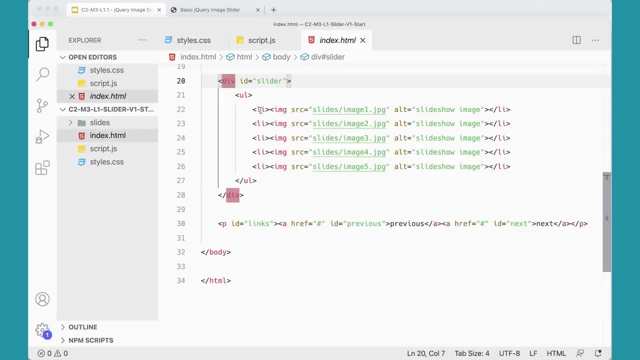 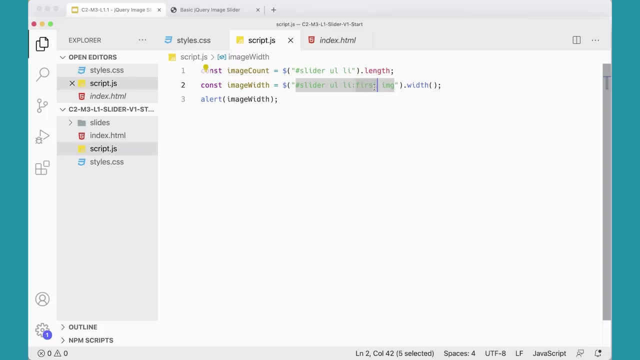 and it looks at the first one of these list items and then gets the image. Now, as it turns out, jQuery has deprecated this first pseudo class. If you look this up on the jQuery website, it'll say deprecated. They don't want to use this. 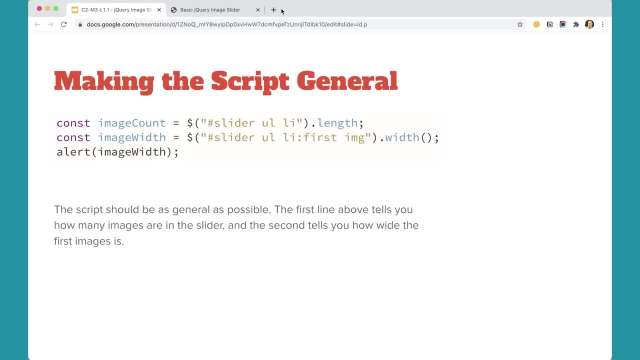 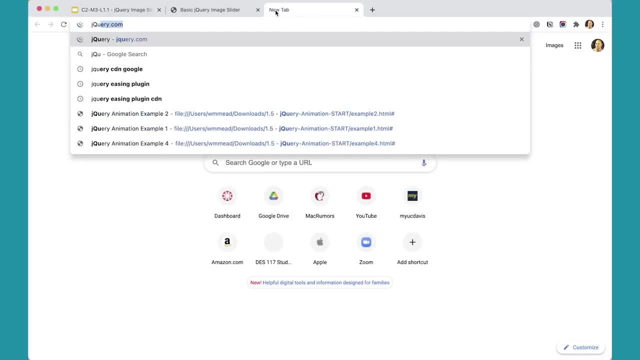 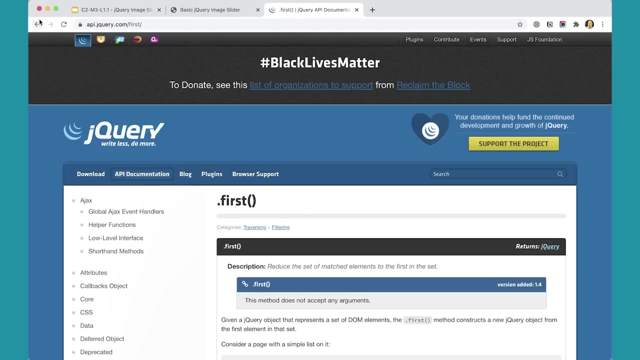 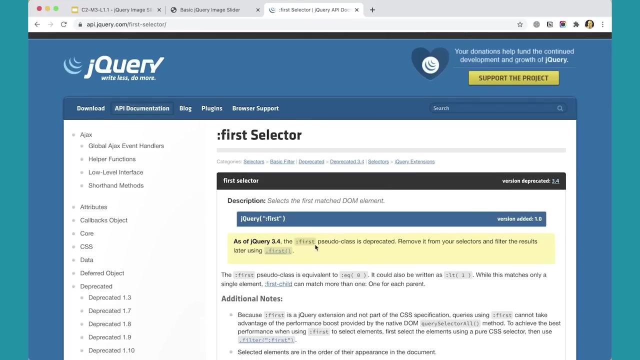 instead they want you to use the, the first method. So let's actually do that really quickly. If I just do first, I'll do jQuery colon first and look up this one. here You'll see. as of jQuery 3.4, the first pseudo class is: 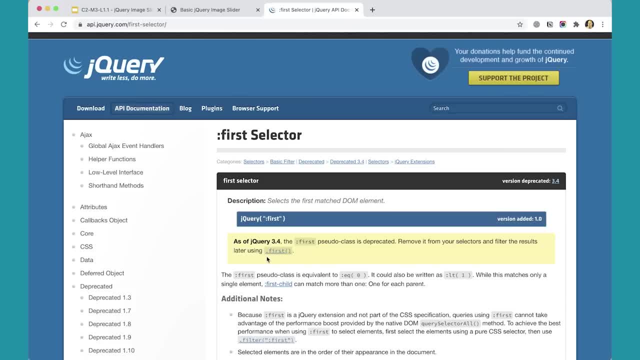 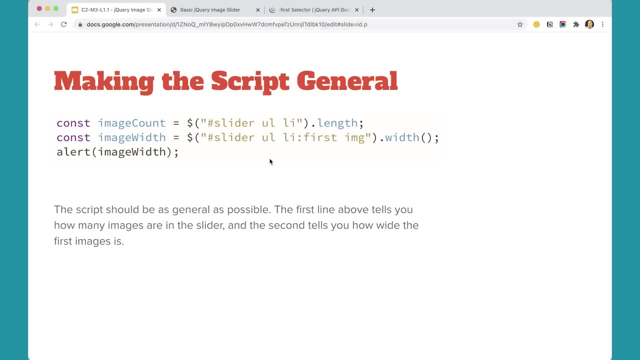 deprecated, Remove it from your selectors and filter results using dot first instead, And it's important when you're using a library like jQuery to stay up on sort of the latest trends with the language as best you can. It's not always easy to This one slipped by me when I made this slide, but I'm aware. 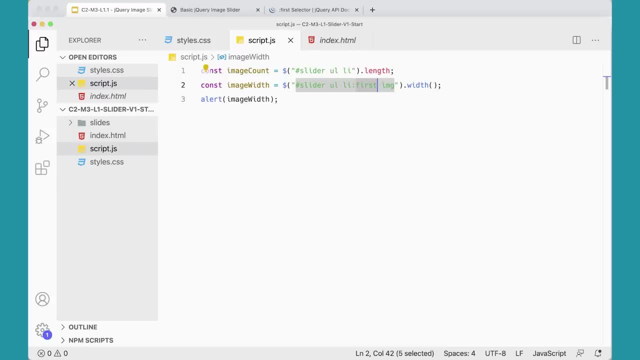 of it now. So I'm going to fix it here in the video really easily here. I'm just going to come over here and get rid of first here and instead use dot first, First, like that, and that should get me the same result. Let's just check, really. 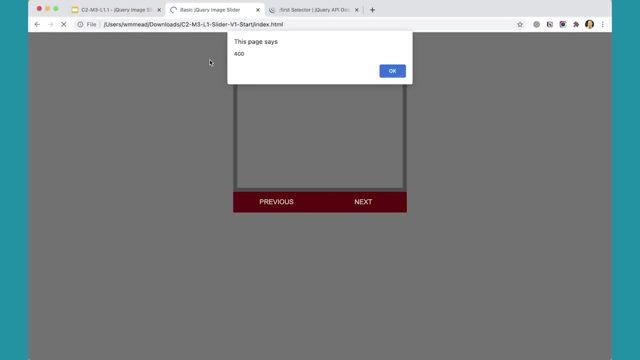 quickly. I come over here and refresh the page. I'm still getting 400, so that's great. So it is important to sort of pay attention to these things as you can. I should add, while this still works currently, in the current version of. 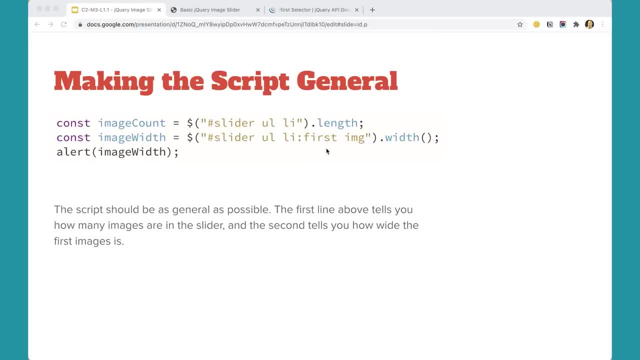 jQuery. it might not work in future versions of jQuery And since I'm loading this version of jQuery up with this project, unless I update my link to jQuery to a newer version, it will continue to work. So this is actually fine to use for now with the current version of jQuery that we have. 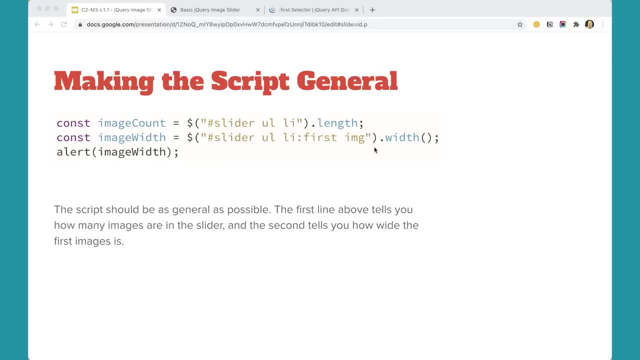 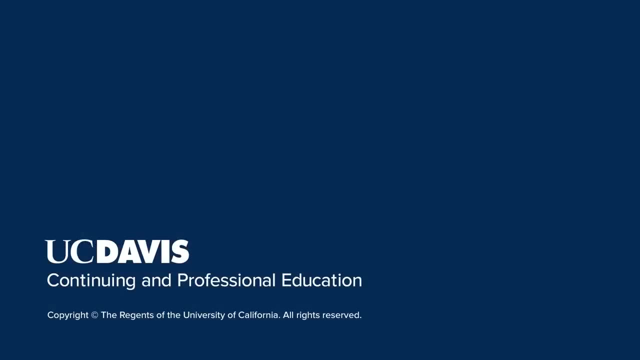 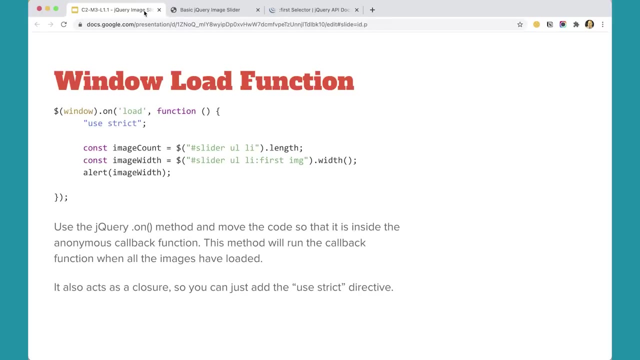 But going forward, we should use dot, the dot first method instead, And I just wanted to show you that. The next thing to consider is the fact that we're going to be using jQuery for this project, And what we're going to consider is when resources are going to. 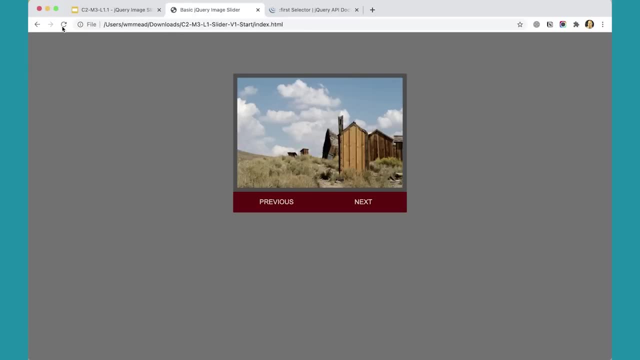 load And in this case this seems to be working just fine. If I click refresh, it's giving me a 400 here, But it's loading these images. Now I have this file local on my computer and that's all well and good and fine, It's going to. 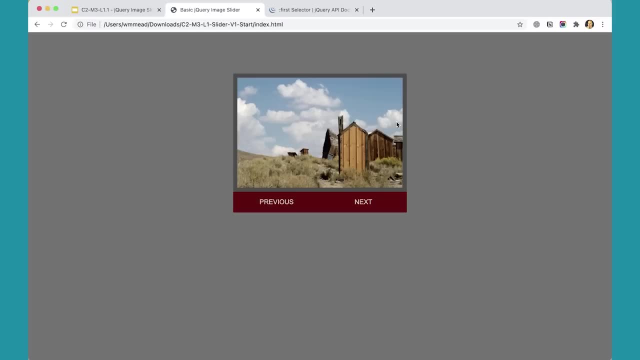 load it really quickly, since it's local on my hard drive. However, if I were actually putting this on the Internet, it's possible that that request to find out how wide the images are would run before the images have downloaded and I could get a zero there. 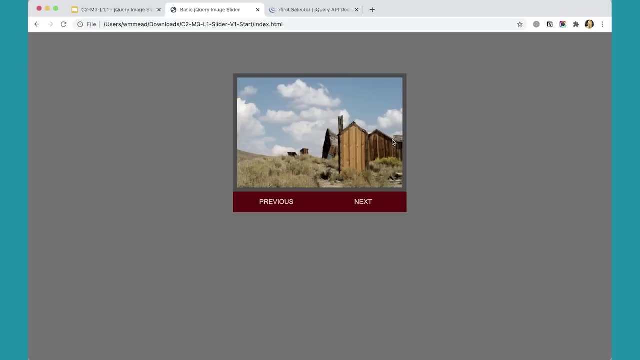 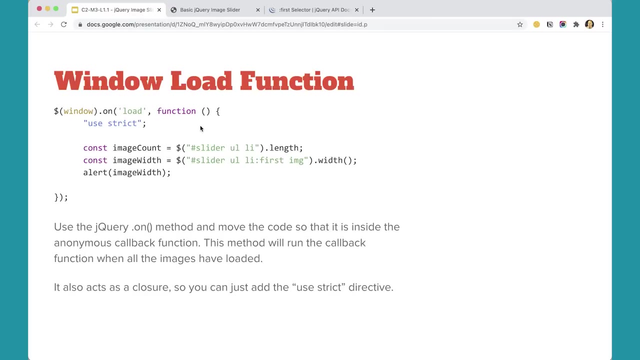 And I don't want that. I want to make sure I'm getting the actual images. So what I want to do to sort of prevent that kind of problem from happening is I want to add an event listener that checks to see when all of the assets for 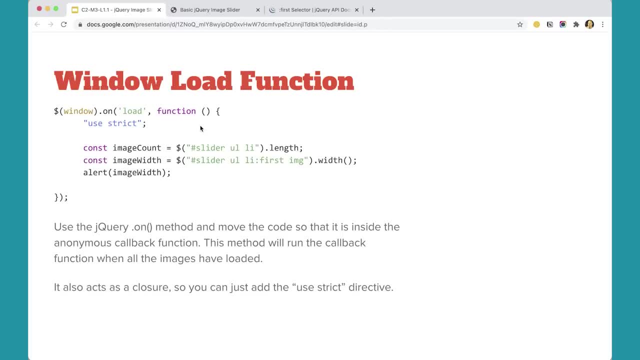 the page have downloaded And it's not going to run the script until they're all downloaded. So we can use the onMap method in jQuery, and the on method in jQuery is similar to the addEventListener method that we have in plain JavaScript And that you pass in a particular event that you're looking for and then it'll. 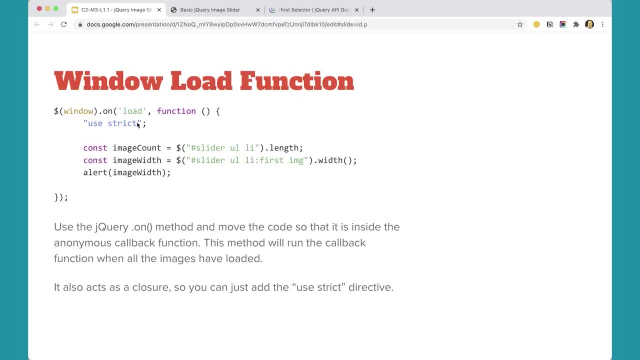 run a function when that event happens. So here we're going to put the on method on the Window object and the window itself And we're looking for a load event And this event, this function here, will run, this callback function will run. 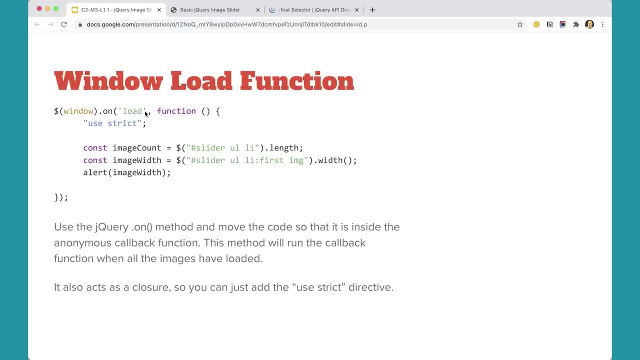 when then load is completed, meaning all of the images for the page have downloaded. So that will keep the script from running until the images are actually there Again, while we're working locally on our hard drive. not such a big deal, But if you put this script up on the Internet, 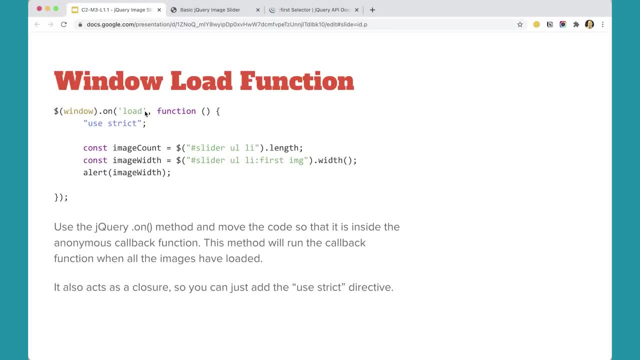 you don't want your slider to think that your images are zero pixels wide, because that will screw up the whole script and that would be bad. So let's go ahead and add this onto our script and we're going to put everything inside this window load function for our page. 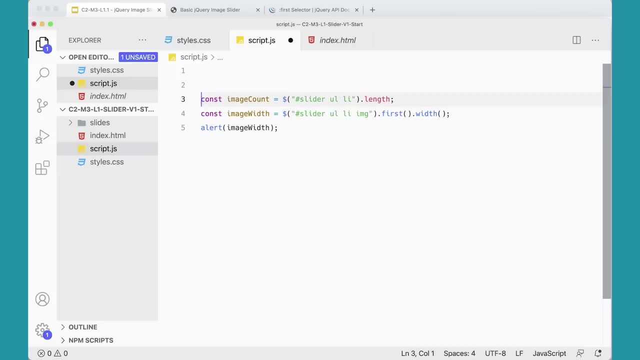 So over here I'm going to add my jQuery object and I'm going to pass in the window object And I don't have to put that in quotes because it is an object. The window is an object that jQuery recognizes And I'm going to use on. 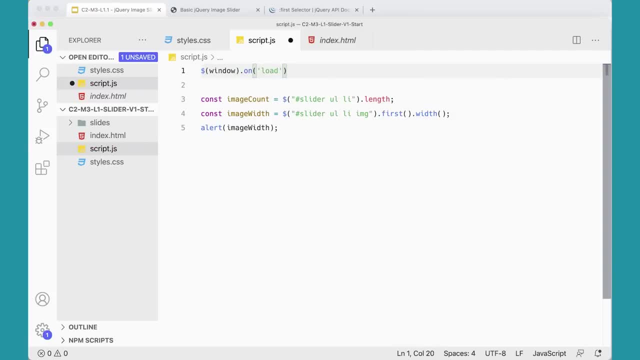 and I'm going to look for the load event and then I'm going to run a callback function Like so, And then everything's going to go inside of these curly braces here So I can actually move all of this up, cut it from there. 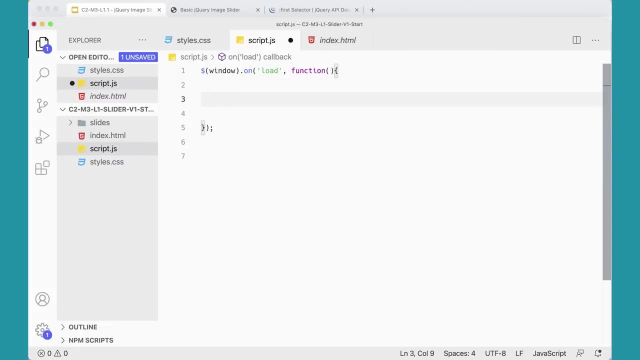 and paste it in here Like that, And while I'm here, this thing, this function here, will work as a closure for the page for this function. So this thing is all in its own closure, So we can add our use strict directive right here. 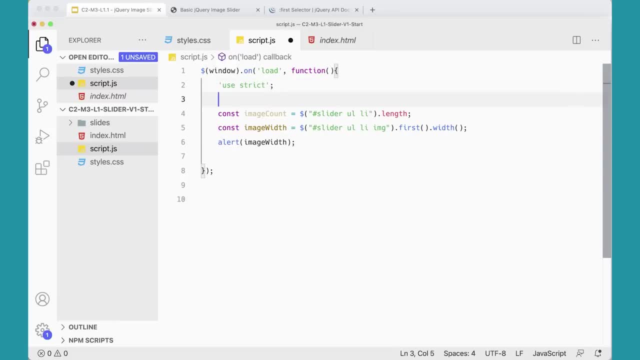 And we don't need to make a separate IIFE- the immediately invoked function expression. We don't need to make a separate IIFE- the immediately invoked function expression. We don't need that because we want this function to run when the page has loaded all its files. 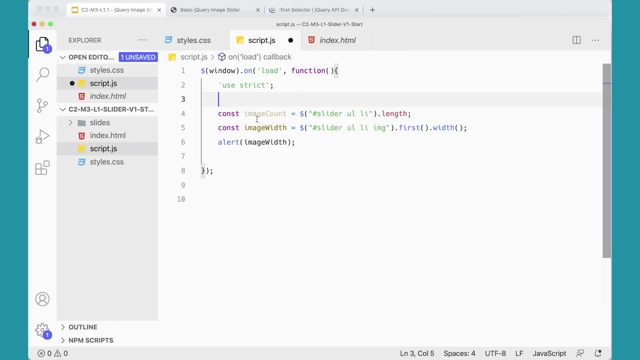 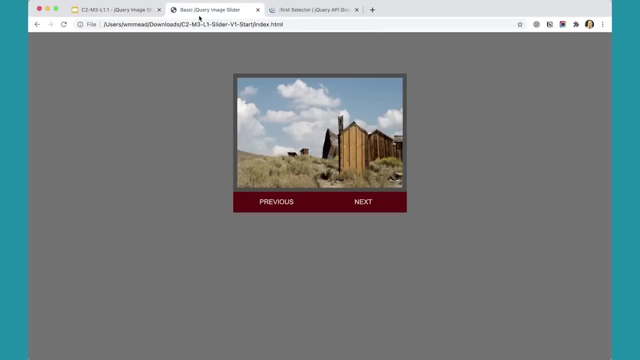 And when it has, then we can say: okay, now you can run And we're going to set up these variables in alert And this should show absolutely no difference at this point over here on the front page, As soon as- as long as I typed it right, we should still be getting 400. 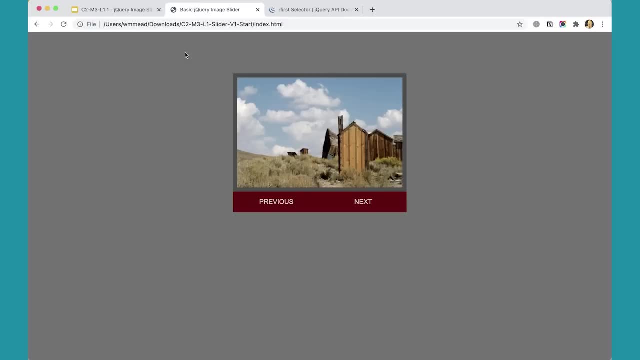 But you can see that the image started actually coming in because before that alert ran. So that's one thing that's slightly different is that it's actually running. So that's one thing that's slightly different is that it's actually running. So that's one thing that's slightly different is that it's actually running. 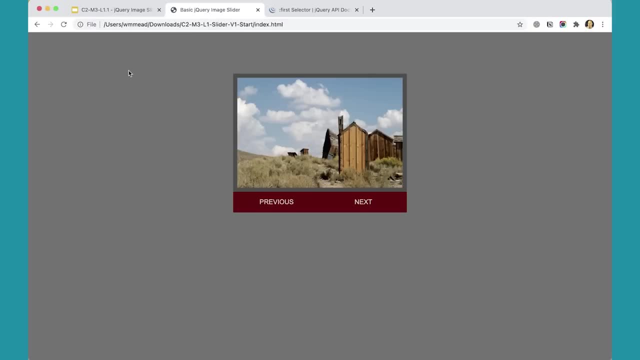 So that's one thing. that's slightly different is that it's actually loading the images first, And because we're loading from our hard drive, it's not that big of a deal, But it's still kind of. it's still a really good idea to do it this way. 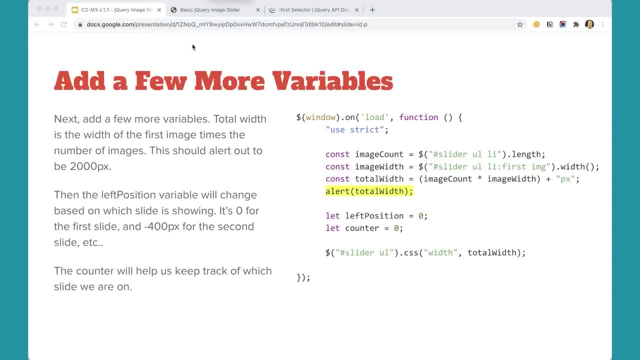 Next we're going to add a few more variables to our project. We need to know the total width of our whole slider, And for that we're going to take the image count and multiply it by the width of each image, And that will give us our total width. 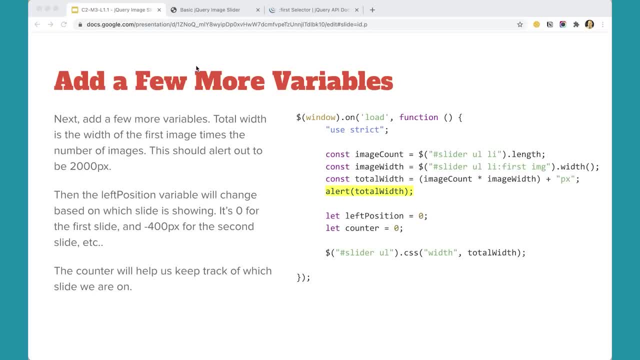 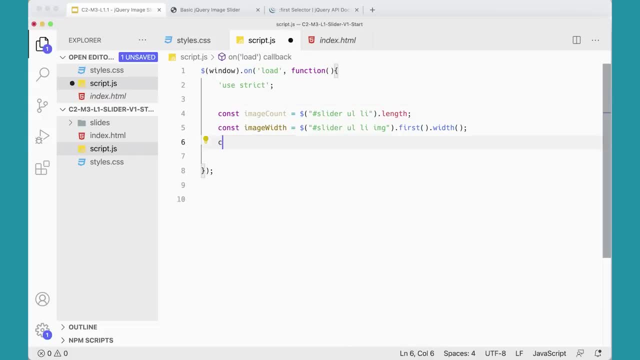 Plus, we'll add a tx to the end of that, So let's go ahead and add that to our script. now I'm going to get rid of this alert and just do const total width, And this is going to be equal to image count or image width times image count. 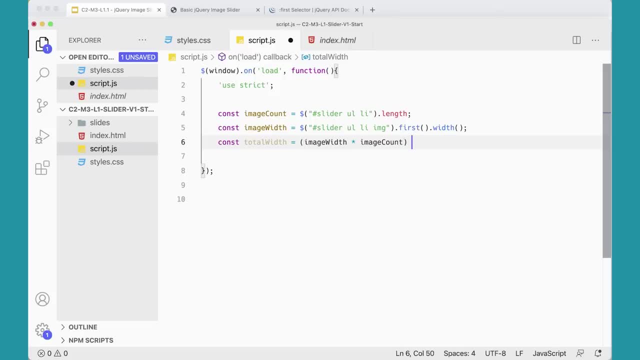 It doesn't matter which way around it goes. right, It's going to come up the same thing, And then we're going to add on to that a px at the end of there. So that's going to put that. put that in there. 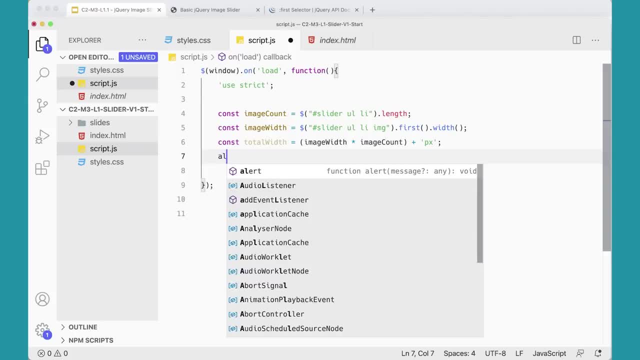 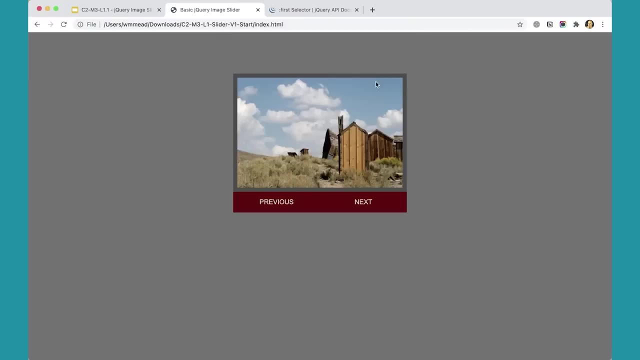 And then let's just alert out total width, Alert total width, just to sort of see what we're getting here. So I'm going to come back here, and now, when I refresh, I'm getting 2,000 pixels because I've got five images. 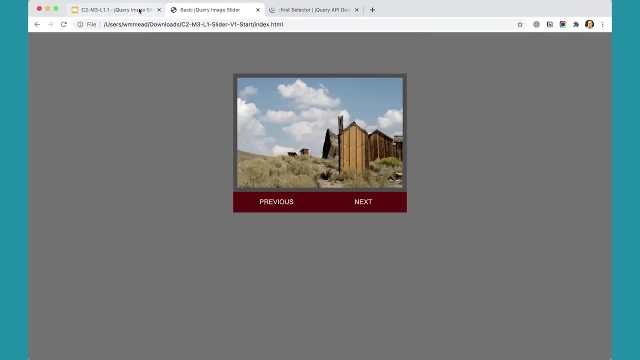 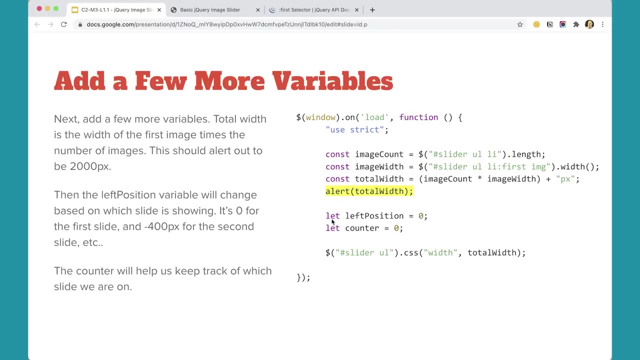 Each of them is one image. Each of them is 400 pixels wide, that's 2,000 pixels. So that's adding up and doing that properly, which is great, Okay. Next, I'm going to need a variable for left position. 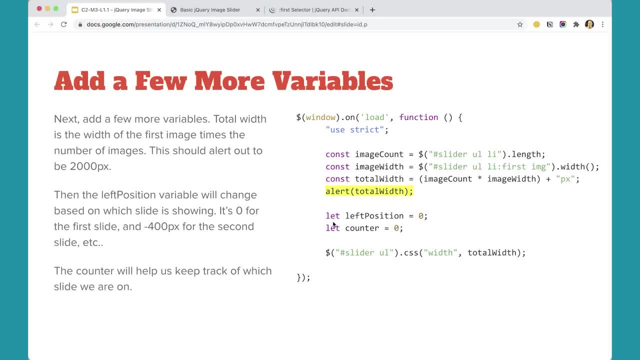 This variable is going to be changed in the process of running the script, So I'm going to set it with the keyword let and I'm going to have a counter that's also going to change. And then I'm going to set the width of my slider UL to be that total width. 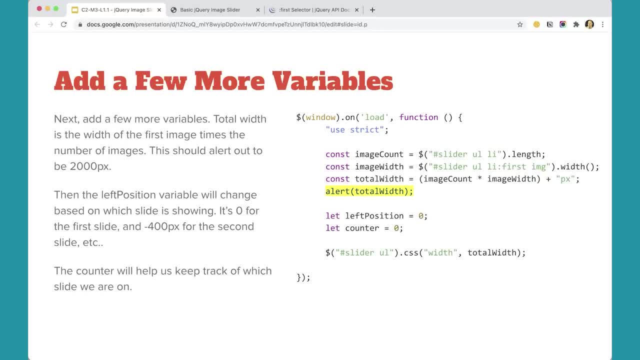 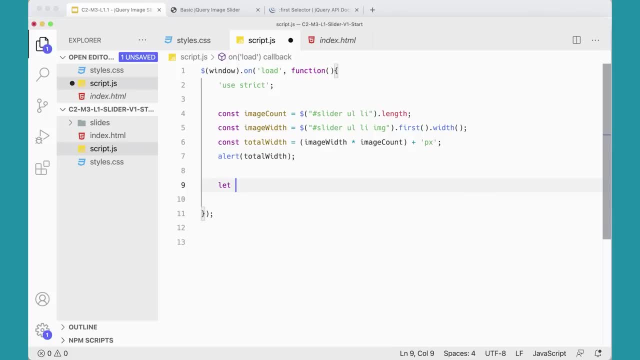 And we'll talk about that in just a minute. Okay, Just a minute here. Let's go ahead and add these in: Let position equals zero, Let counter equals zero, And then I'm going to use my jQuery object to go in and say: okay, pound slider UL. 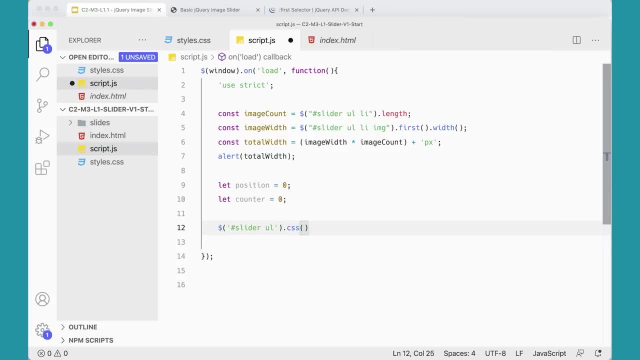 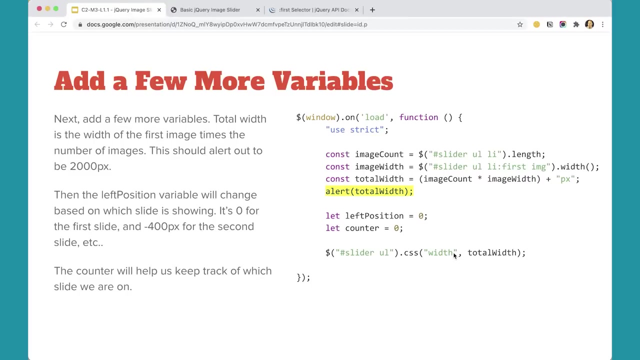 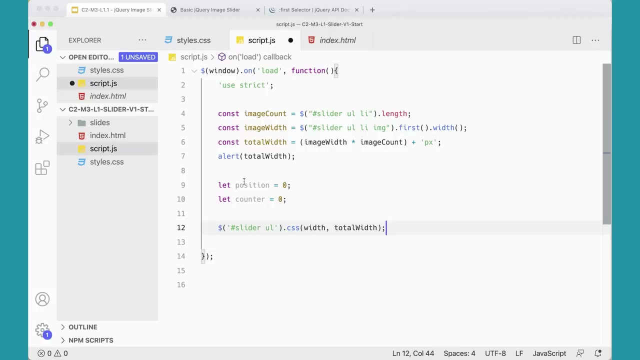 Dot CSS. your width is going to be total width. Did I do that right? Let me go check my slide over here and make sure I did that right. The width needs to go in quotes. All right left position. let me just change that. 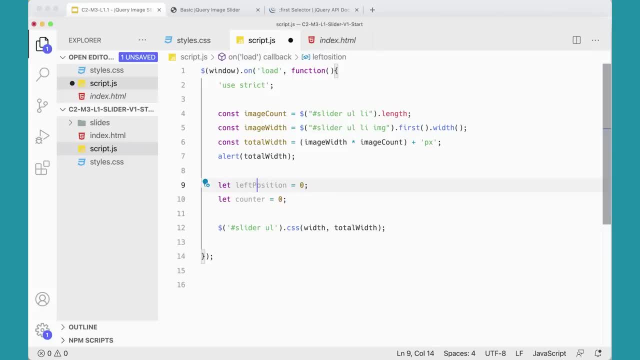 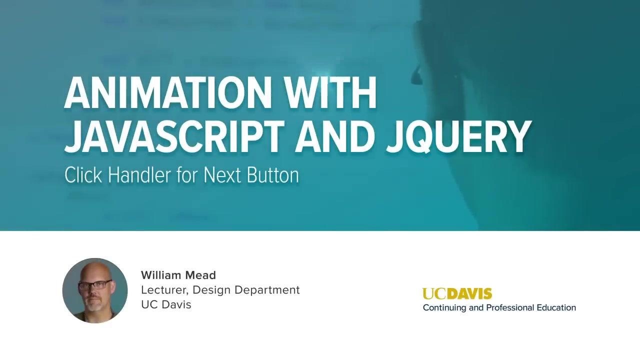 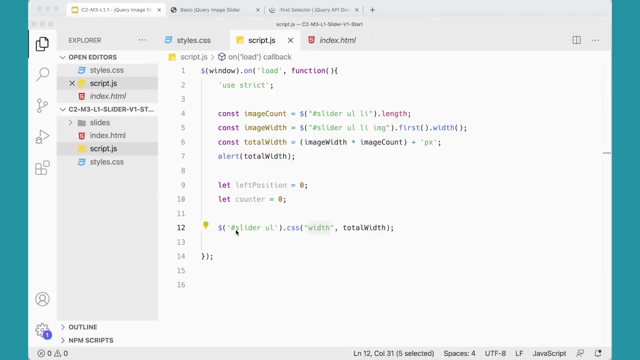 Left position And width needs to go in quotes. And there we go. So let's, let's stop the video here And then we'll talk about this more in the next video. In our previous video we had set this setting here. 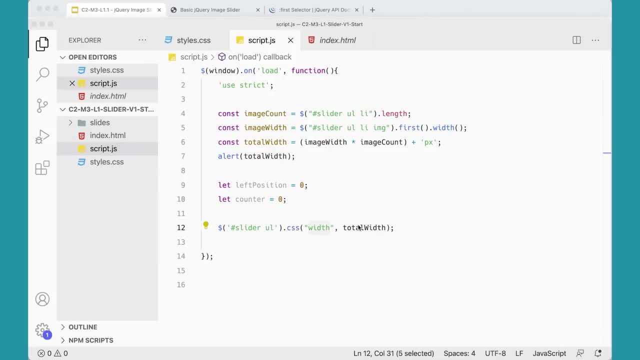 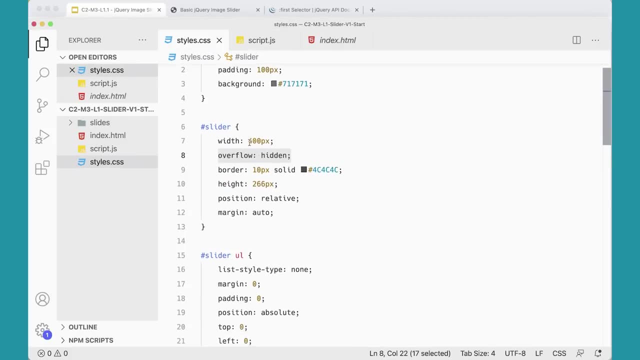 which sets the width of our unordered list to the total width, and i just want to talk about this just for a second really quickly. if we go over to the styles over here, you'll see on here that the slider ul isn't given a specific width, but i want to add a width to it because that will just make sure. 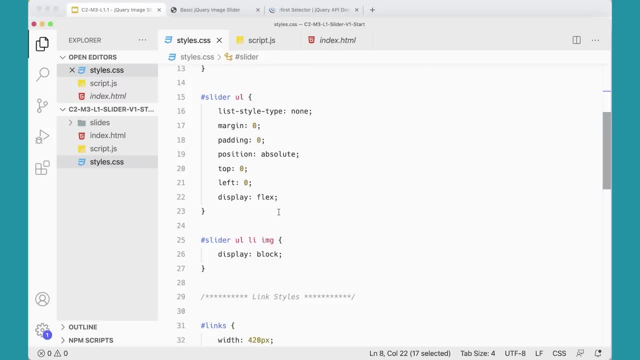 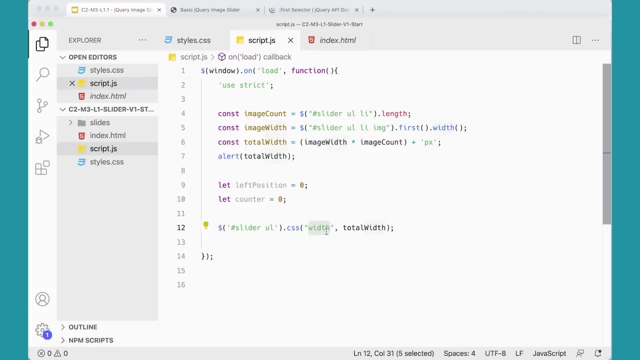 that when i set it to display flex and that every that everything's going to fit properly inside this ul. so this adding that to the script just ensures that the slider is going to be the exact width that i need it to be- 2000 pixels. i don't really need this alert to come up anymore. 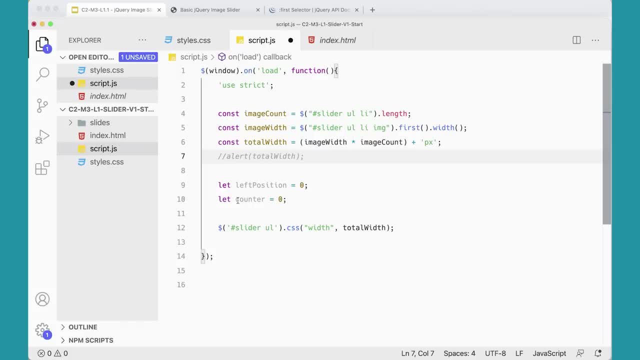 so i'm just going to comment that out. but that gets us all kind of set up with all our variables that we need in order to get started with this script and get it working the way we want it to work. now we're ready to add our click handlers and actually make the script actually work. 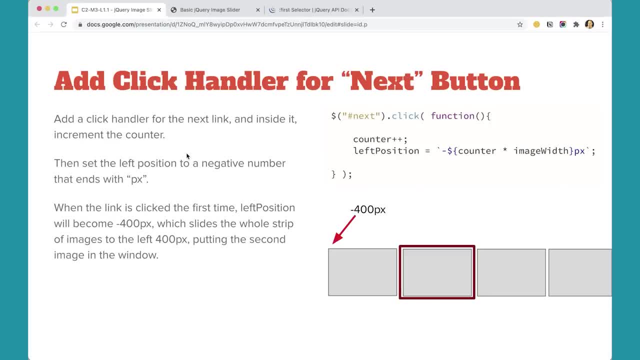 so let's go ahead and do that. so we need a click handler for that next button, and when you click the next button, we're going to increase the counter. so the counter is going to go from 0 to 1, and then we're going to set the left position to a negative 400 pixels. 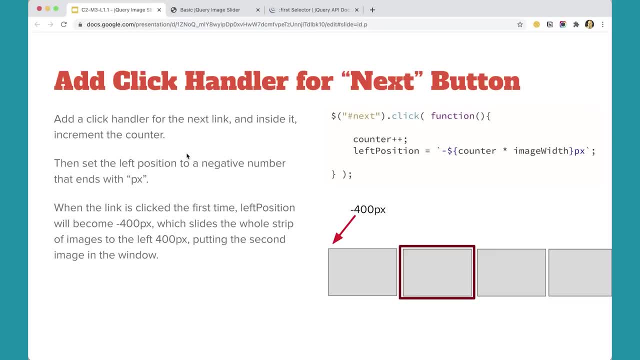 so we take that counter and we multiply it by the image width: 1 times 400 is 400 and we're going to put a minus sign in front of it because we're going to move it a minus 400 pixels. so let's go ahead and add this into our script over here. 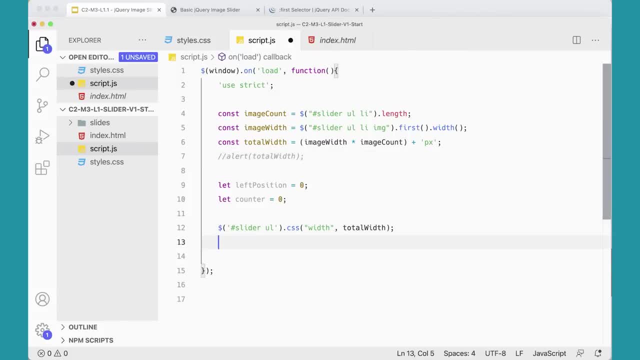 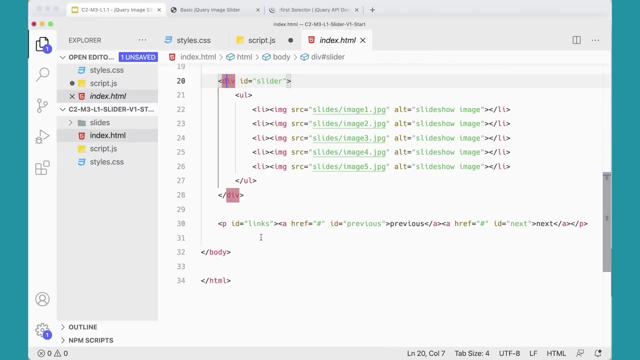 again, the best way to do this is to type from the outside in. so i'm going to add an event listener like this: i'm going to start with my jquery object and then i want to get the element that i want to work on, my pound. next element, which, if we go back to the index file here, is this link right here: id. 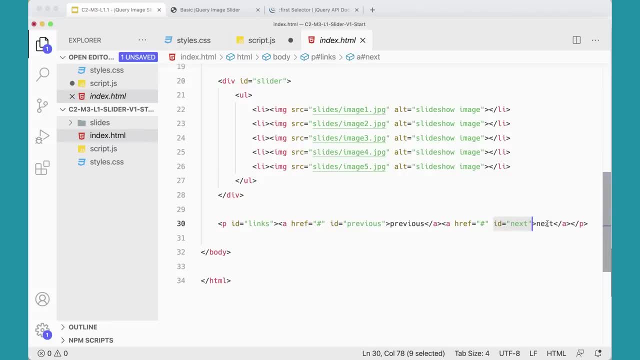 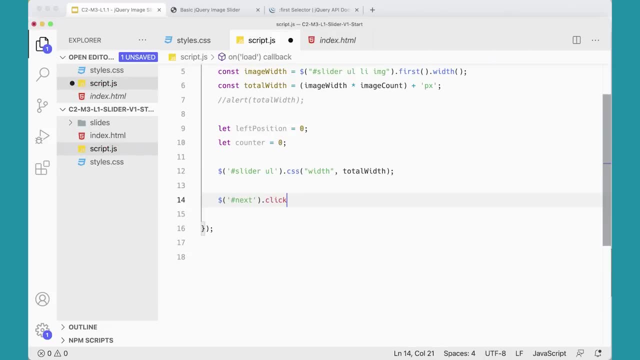 equals next this link. when you click on this button, it says next: so when we click on that, we want to have a click event handler like so. so when you click on it, you're going to do a click and then we're going to pass in an anonymous function that runs when you click. function. 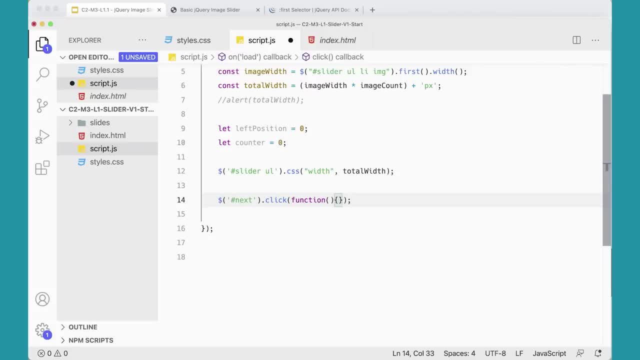 parentheses. curly braces. click between the curly braces and move that down. all right, so when we're here now, we're going to take counter, which is the variable that we created just a minute ago, counter, and we're going to increment it plus plus. so counter is now gone from zero to one and we're going to set the position of the um of that slider. 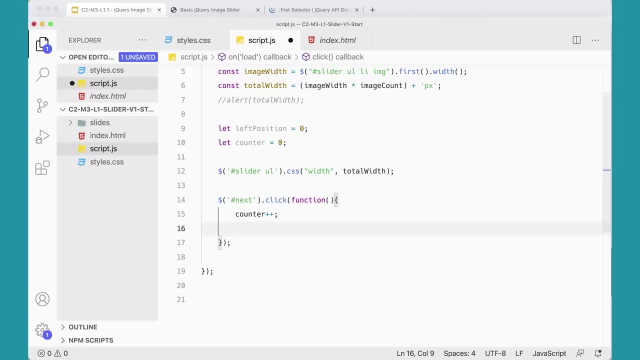 over to the left minus 400 pixels. so we'll set left position. that variable there is going to be set to equals. what did i do here? i need counter times, uh, image width- and i need a negative number. counter times, image width- a negative. so that's going to give me a. 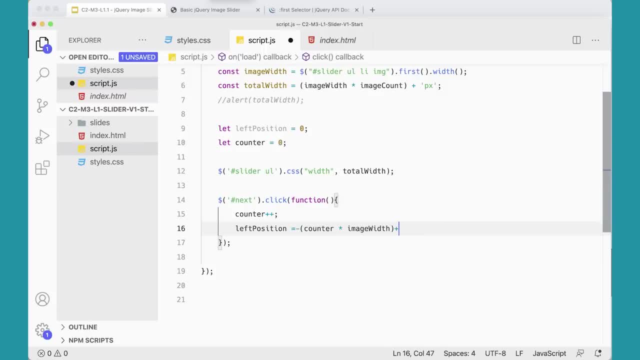 negative 400, and then i also need plus px, i believe, and that will set that left position to what i, what i needed to be there split. now i see i did the right thing there. i want to write. well, this should work. i think it's a little bit easier to read if i use my tick marks. 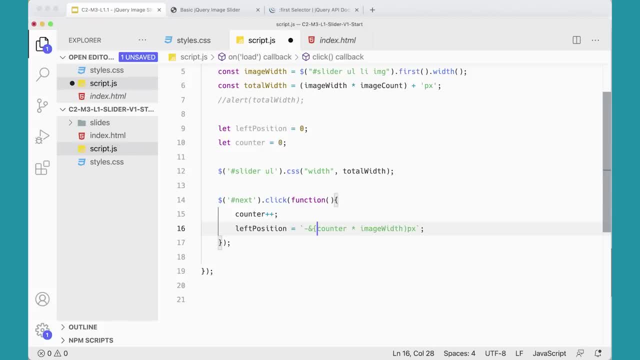 the dollar sign and the curly braces- oops, dollar sign and curly braces, like that. so i've got counter times, image width. so i'm using my string literal here to get to give me a negative to counter. multiply by image width, that's going to generate a 400 and put a negative there and put: 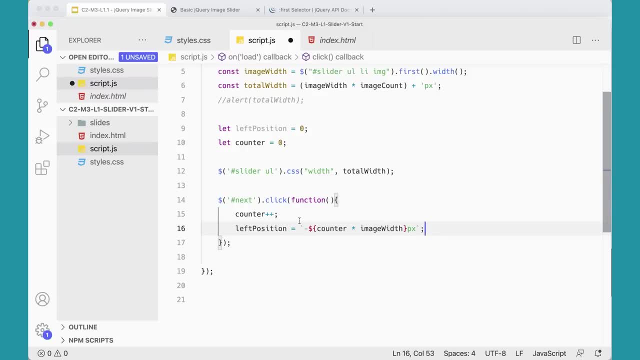 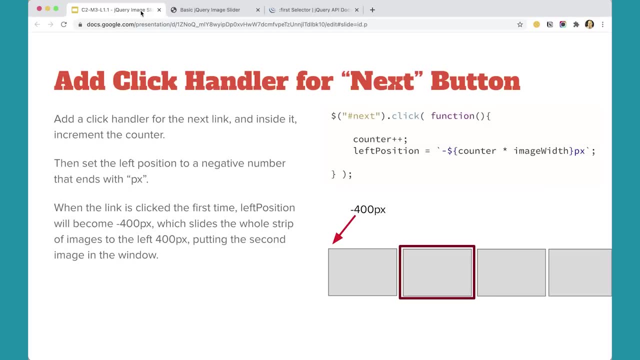 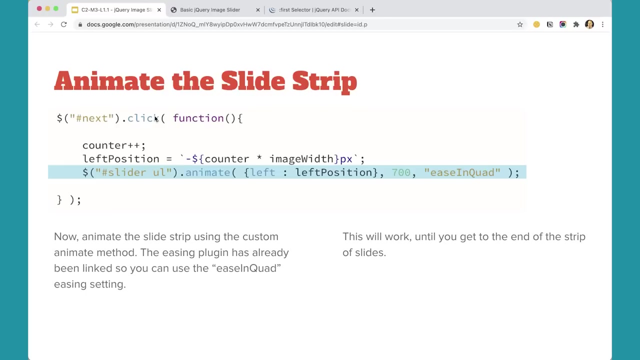 a px there. so that's great. so there we go. that's going to set the left position. now all we need to do is to actually animate that element, and what will that look like? it'll look like this: we're going to go get that slider ul and we're going to use our animate function and we're going to 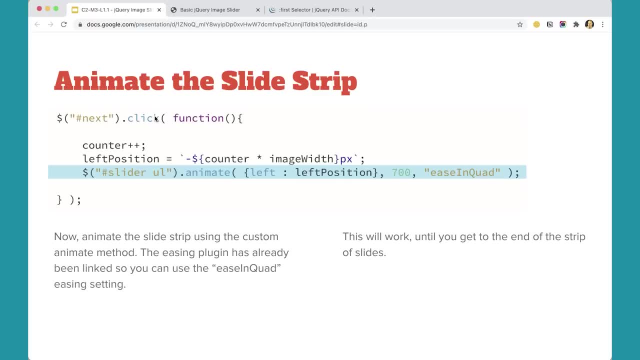 animate the left property to left position, which we know is going to be. when you click it the first time, it's going to be minus 400. when you click it the next time, it's going to be minus 800. you and you click it the next time, it's going to be minus 1200. it's going to move over 400 pixels each. 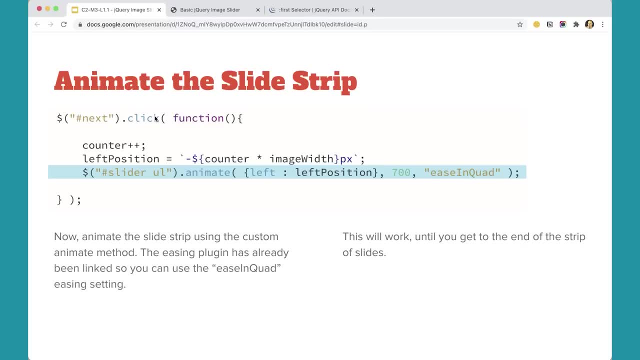 time for each image. we'll set it to a speed of 700 milliseconds and then we'll use the ease in quad easing. and we can use that because we have the ease in plug-in already put into the project. so let's go ahead and add this into our script over here. so down here i'm going to say: okay, great. 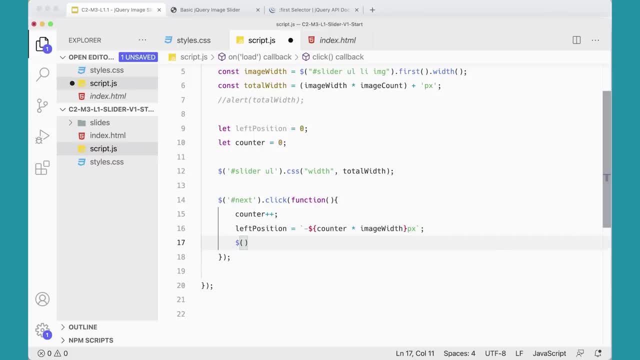 go ahead and get our pound slider ul and we're going to do the animate method on it, our custom animate, and in there we're going to pass in an object. and we'll get more into objects and how they work in a later lesson, but for right now it's just. it just takes key value pairs. we're going to animate the left. 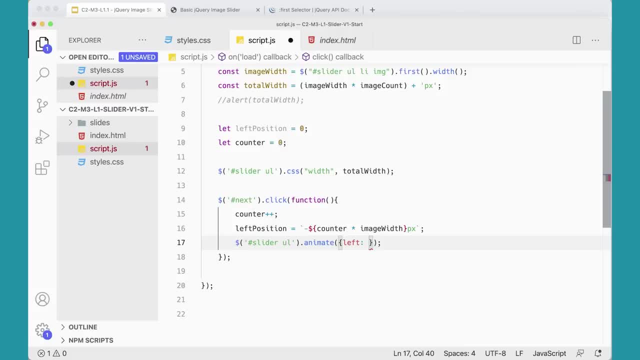 property, and what are we going to animate it to? we're going to animate it to left position, which the first time you click the button will be minus 400, then a comma, and then i'm going to: actually no, we're going to leave that like that. and then, after the curly braces, i'm going to say: 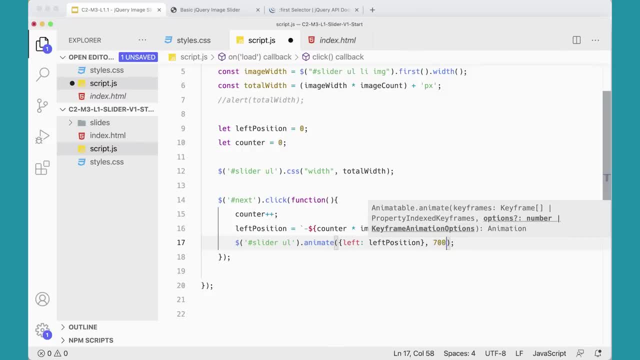 700, because that's the only property i'm actually going to use. that's the only property we're going to use, and then we're going to use the next one, which is the animation, and i'm going to use the animation and i'm going to use this one. 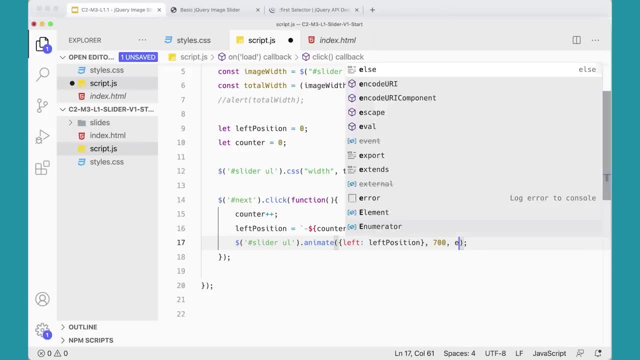 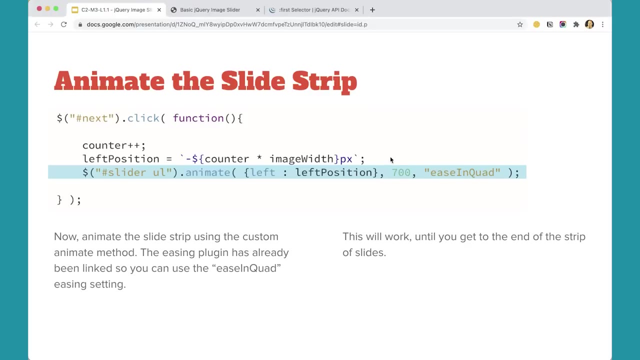 because it's actually an animation. 700 milliseconds is how quickly it's animating and i'm going to do ease in quad, which is the easing that i have selected for this particular animation. you could do a different one if you wanted to, but that will get the correct animation. 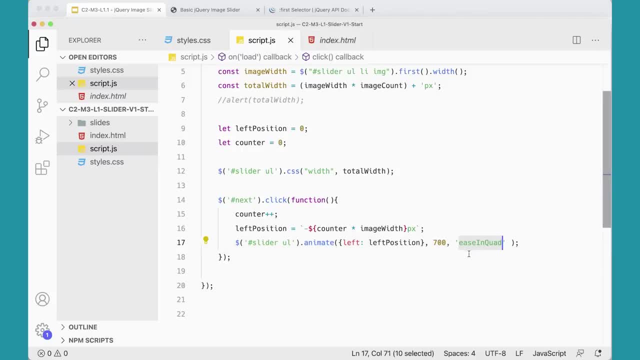 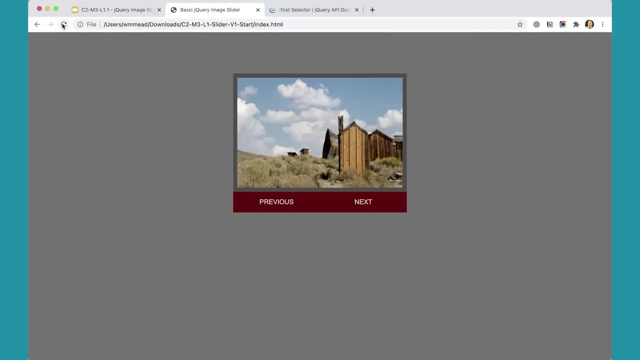 needs to go in quotes like: so now, with that, this should be somewhat functioning. it'll function until we get to the end of the end of the strip, but let's give it a try over here and see if i did it right. so now, if i refresh and if i click next, look at that, it's animating right to the 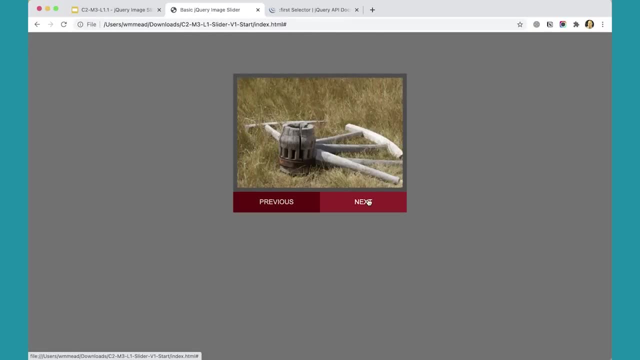 correct spot and then it goes to the next one, and then it goes to the next one, and then it goes to the next one and if i click it on the last one, it animates right outside of this, out of the side of the strip. so the entire strip is off to the left over here. so that's what we'll need to fix next. 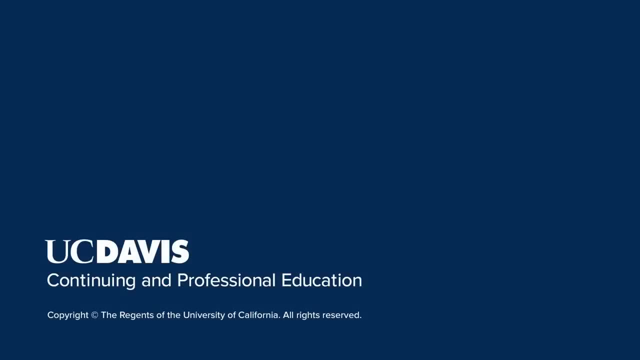 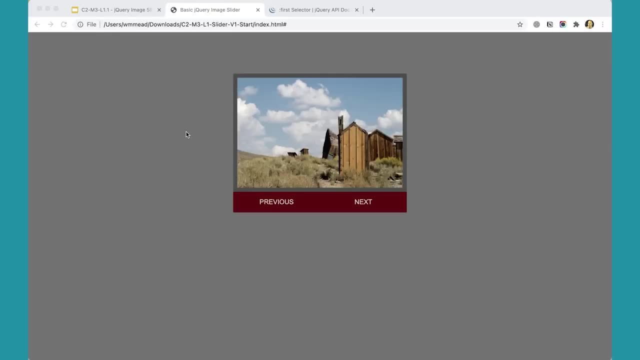 in the previous video we got our click handler working so that you can click on the button and the images will move forward and the slider will function. but when you get to the end of the strip you'll see that it's animating right to the left of the strip. so 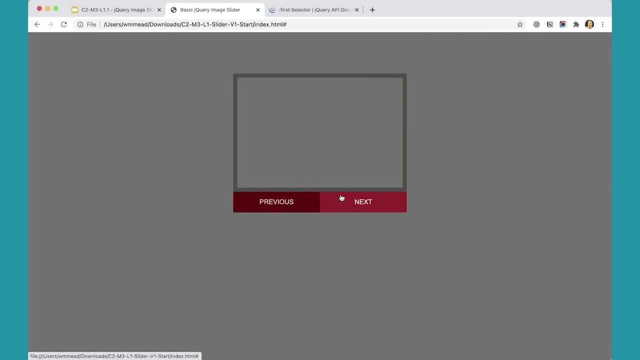 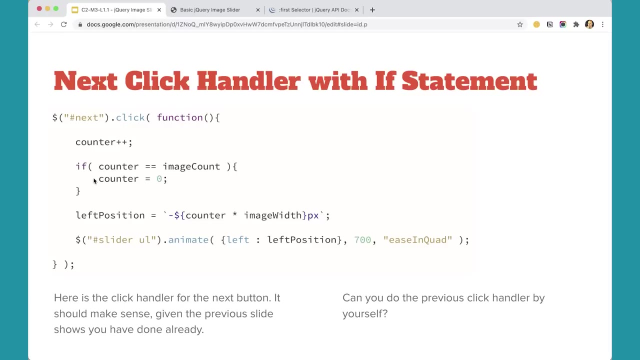 when you get to the end, the strip slides right outside the slider window, which is not really what we want. so what we need is an if statement to make this work. we're going to add an if statement to check to see if the counter is the same as image count, and if it is, then we're going to set. 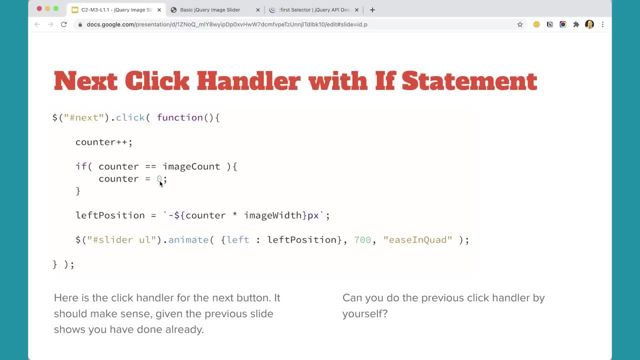 that counter back to zero and that'll put the strip right back to the beginning. so what we want is remember: image count is saying how many images we have. so it's five, so we want a number. that's: either we want counter to either be zero, or we want counter to be zero, or we want counter to be. 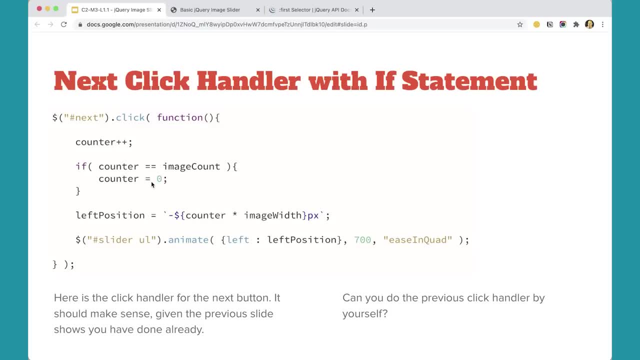 zero, one, two, three or four. as soon as it hits five, then we're out of range and we want to put it back to the beginning. so let's go ahead and add this if statement into our script over here to handle that. so down here i'm going to. 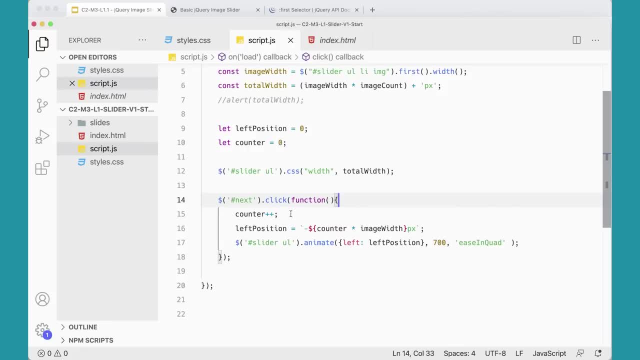 increment the counter and then check to see if the counter- if counter- is the same as image count. if it is, then i'm going to set the counter back to zero. equals, equals. the same as you could also do triple equals, which would be exactly the same as this can. in this case, i'm not really worried. 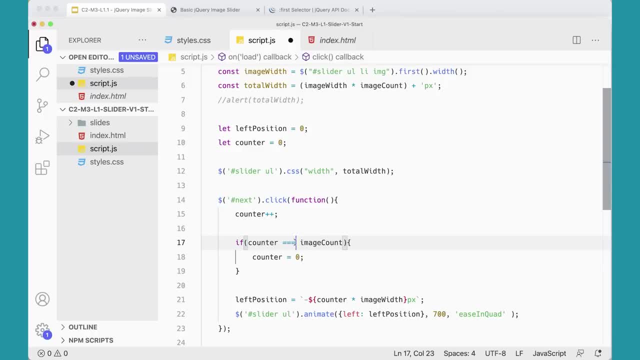 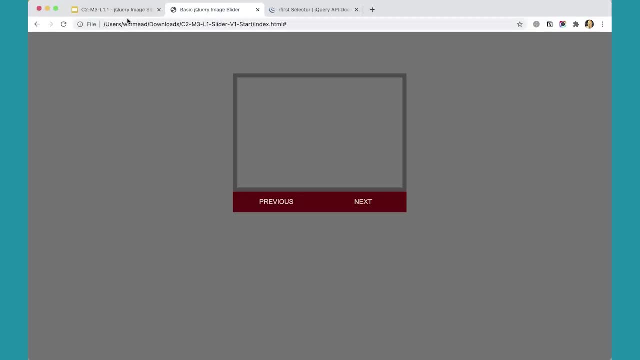 about uh type coercion, but you might want to be extra careful and put triple equals in there. and there we go. so now, if we come back and test this, refresh the page and i click next. it'll go all the way through my slides and when i get to the last one, 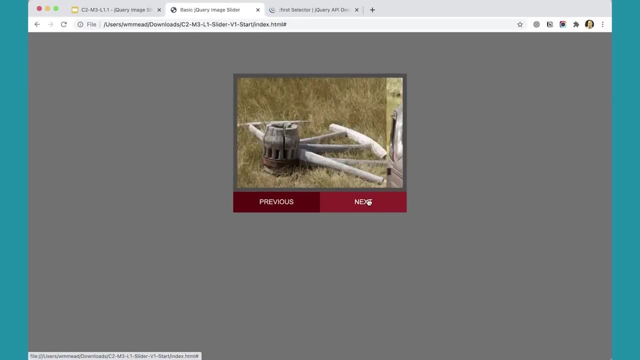 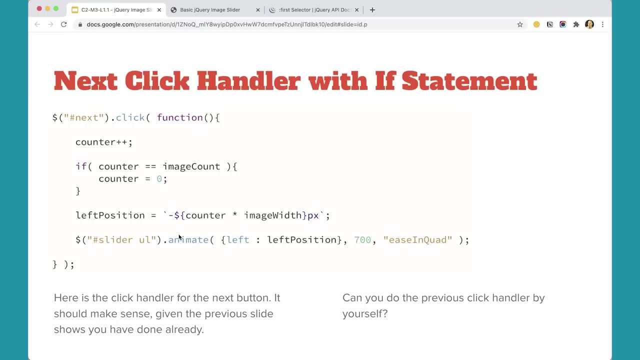 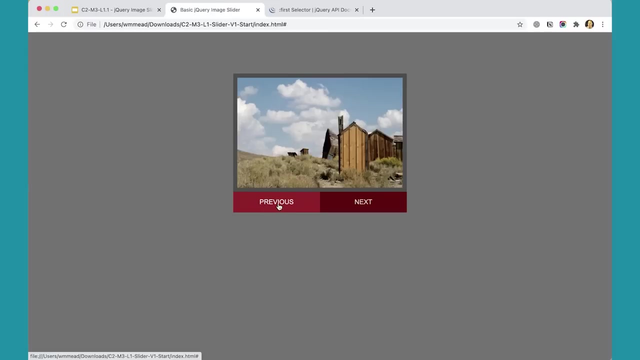 it goes back to the beginning, and that will continue to work as we go forward through the script. great, so now your job is to think about what you could do to create the click handler for the previous button, because currently this button doesn't have any anything going on with it here. it doesn't have any event listener at all, so we need to add an. 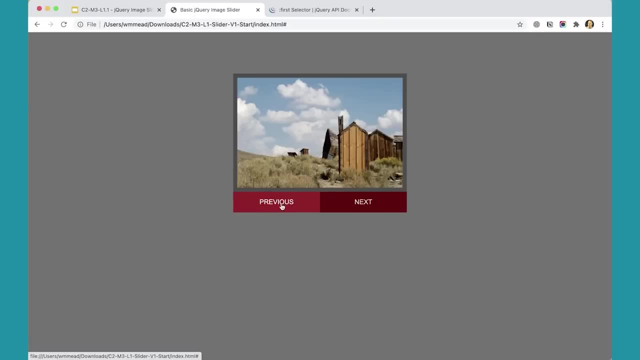 event listener for this. that will make the slide strip go the other way. now the way to think about this is to start with thinking about what happens if you're at the end. whoops, i went too far. there we go if we're at the end of the strip and we click previous. 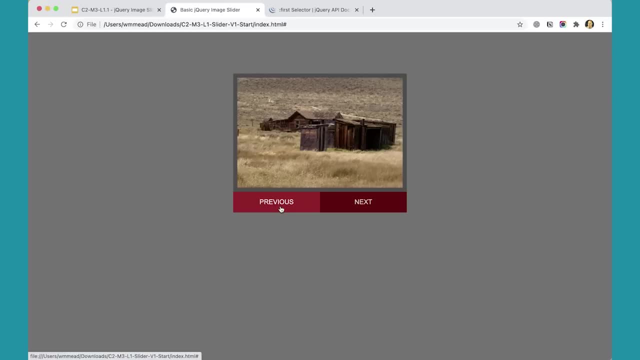 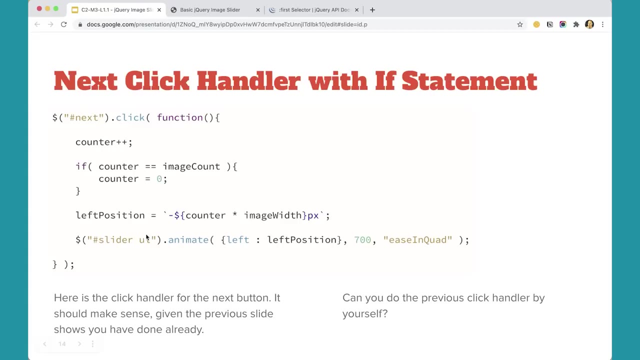 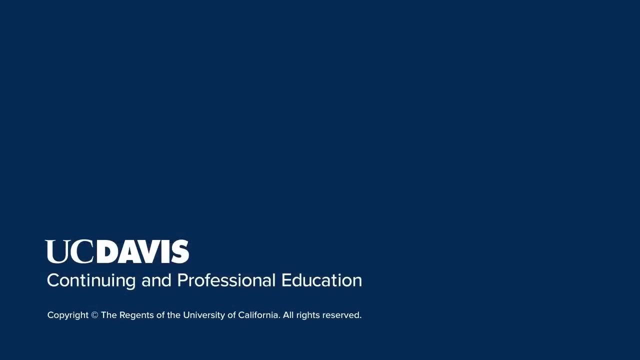 we want to decrement the counter and move the strip the other direction. so think of what you could do to create your own event. listener for the previous click button and then we'll take a look at it together in the next video and see if you got the same answer. 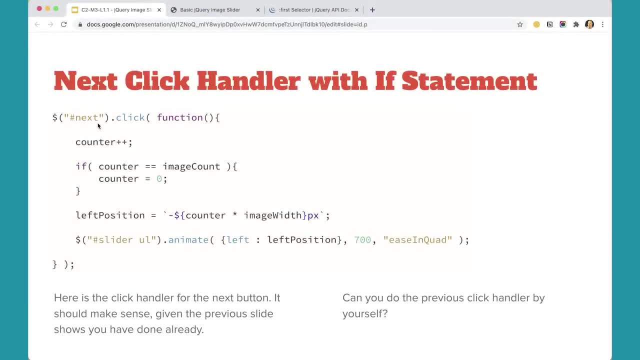 i got. in the last video we created the click event handler for the next button button And it's your job to create the click event handler for the previous button, And hopefully you were able to do that, or at least tried. The only way you're going to learn JavaScript is to 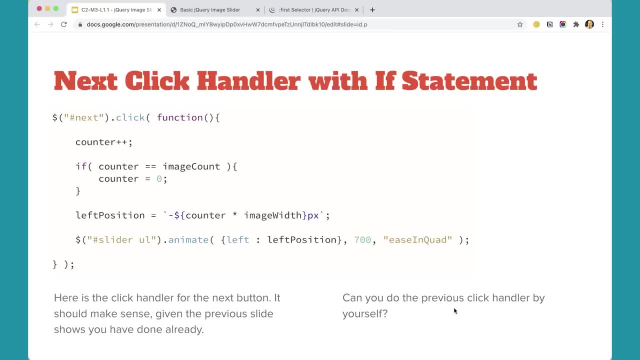 push yourself to do these things without just looking at the answers, and try to do it. Even if you're unsuccessful, that's a success because it makes you think about it, It makes you work with the syntax. So try to do it on your own and then look and see if you got the same answer. I 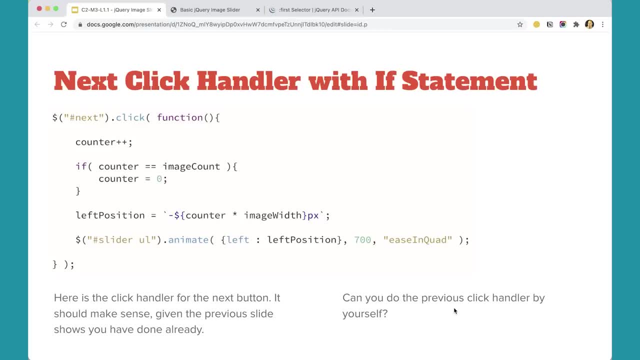 did or if you got stuck, that's fine. You can look and see what I did and hopefully then it'll make sense and you'll have an aha moment. But you won't have the aha moment if you don't even try. 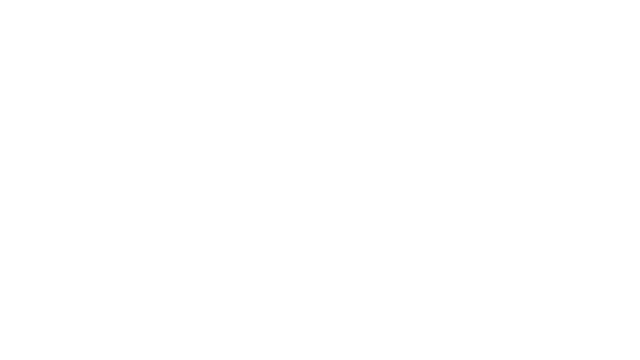 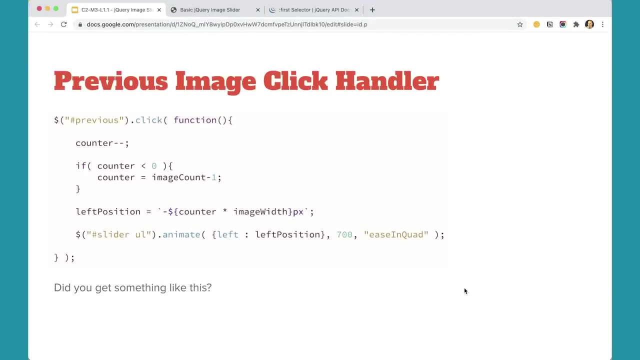 You just look at the answer without trying. This is the answer I came up with. I have an event handler looking for that previous button and for a click on that previous button, And then I'm going to take the counter And here the if statement is going to change so that if the counter is less than zero, then I'm 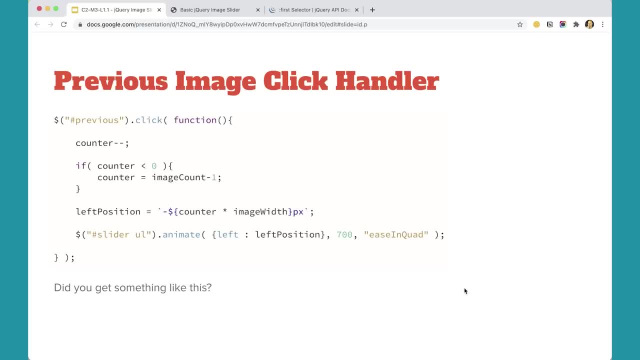 going to set the counter to image count minus one. I don't want to set it to five, I want to set it to four because, remember, our counter needs to be a zero, a one, a two, a three or a four for our 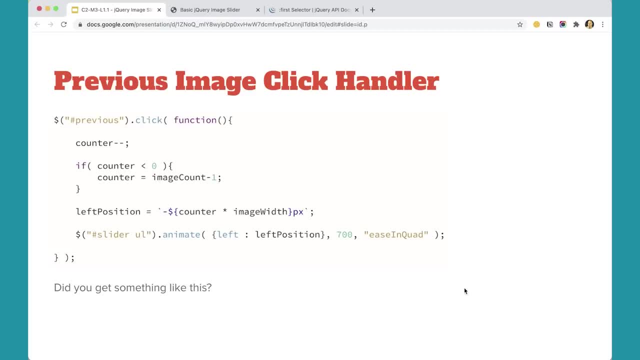 five images. Okay, Those are the four numbers. The five numbers of the counter should be a zero, a one, a two, a three or a four. So if the counter is less then zero, then it's out of range. And then we want to put it in range by putting it at the end. 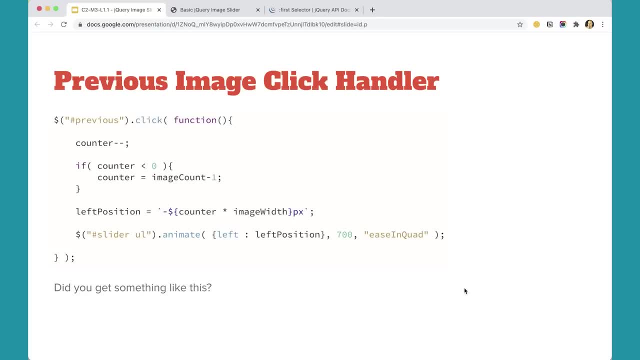 of the strip And then really the way to think about it is to think about it from the right end of the strip, the right hand end, our fifth image, So that if we're on the fifth image we're going to decrement to four, and then we're going to decrement to three, and then to two, and then to. 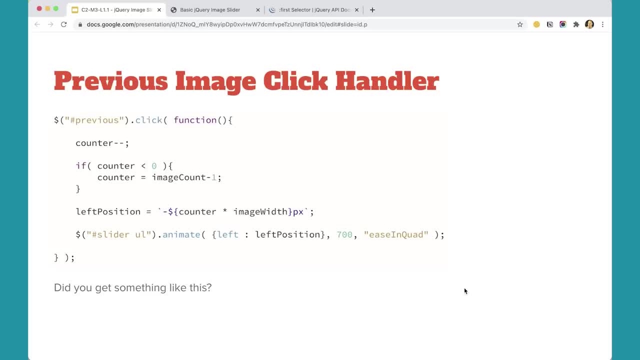 one and then two, And then, when we get to under zero, we're going to set it back to the last image, Okay, And then we're going to leave the left position. These two pieces stay exactly the same. So in fact, we could actually make this script, make this event handler, by copying and pasting. 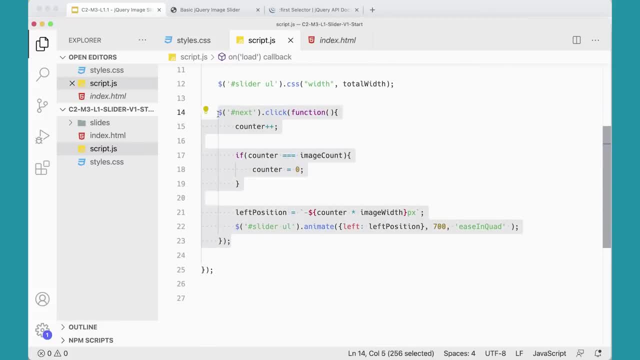 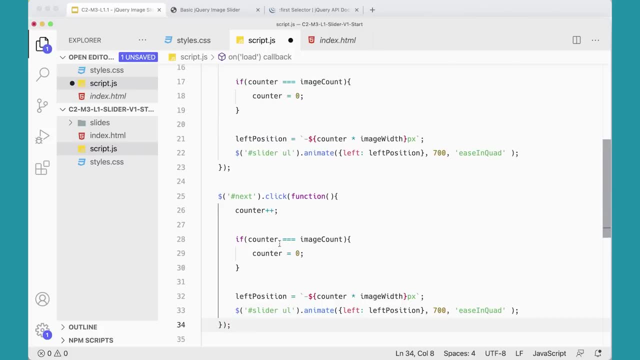 this one, because a bunch of it is the same- the last two bits. I'm going to have to type that again. We can just copy this and paste it And then what we're changing here is, instead of next, we're changing this to previous. 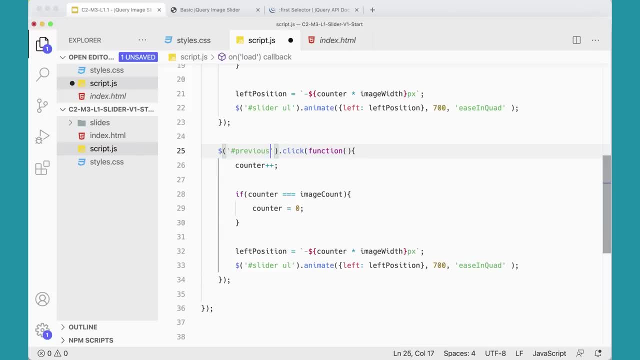 Ideally, we want to do less typing, if we can. The counter, instead of getting incremented, gets decremented, minus, minus, And then, instead of setting counter checking to see if it's the same as image count, we're going to see: is it less than zero? 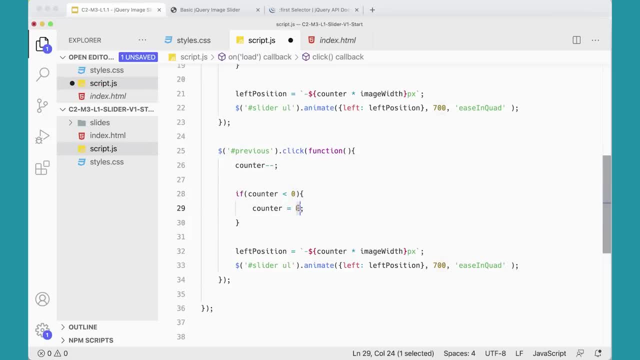 If it's less than zero, then we're going to set it to image count minus one. Remember, we're talking about an image count. We're not going to set an array here. We want our counter to be a zero, a one, a two, a three or a four. 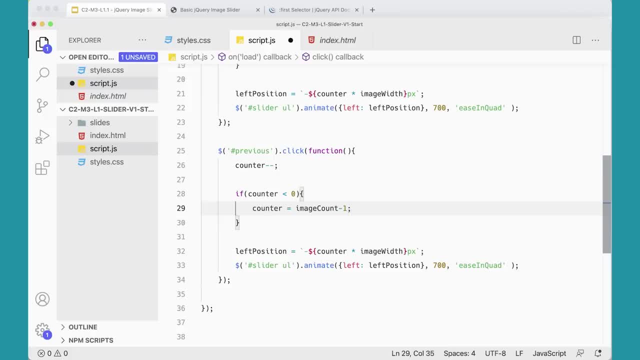 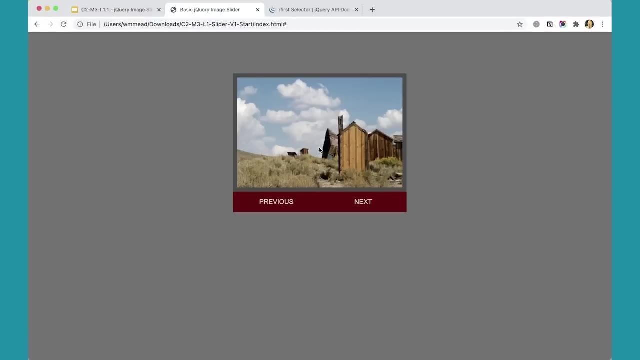 But when it's five that's too high. So image count is going to be five in this case. because we have five images, There we go And then these two remain the same. Let's test it and see if that works. Come back here. Refresh the page. Our next button works. 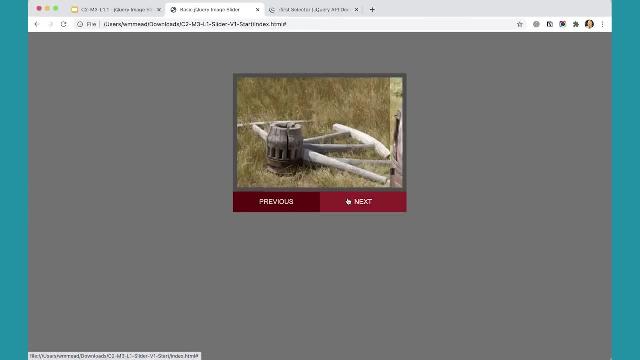 Our previous button works. So if I go all the way to the end, I can go all the way to the beginning. If I'm somewhere in the middle here and I click previous and then click previous again, it will go all the way to the end. 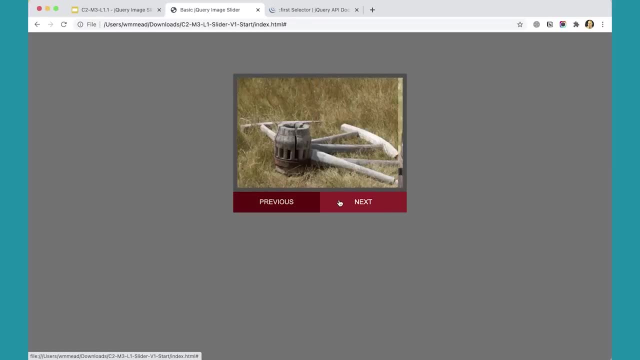 And there we go, So I can go next and previous and I can go And basically this is a strip of photos that's moving back and forth inside of this window And that's working great. So here you have a basic image slider that you could style and work with images on your website, for any website you want. 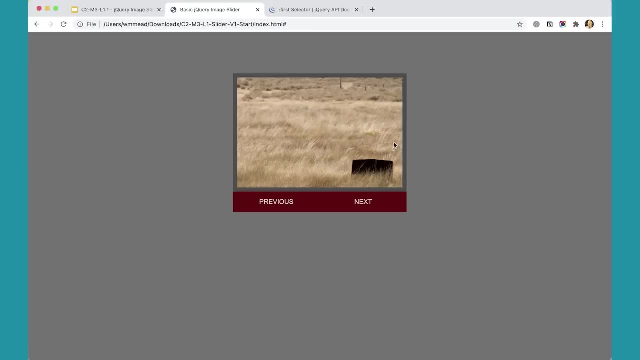 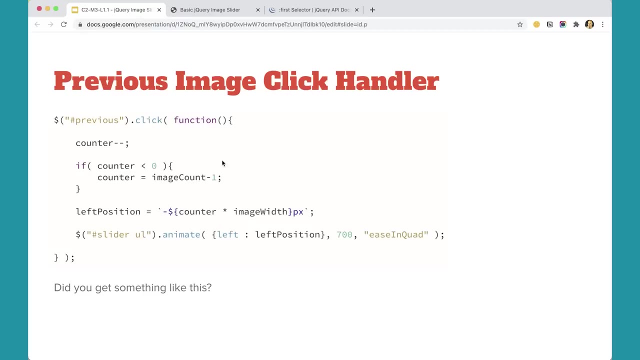 You just want to make sure that your images are all set up to be the same size to begin with, and it'll just work, And you could have as many of them in there as you want or as few of them in there as you want. 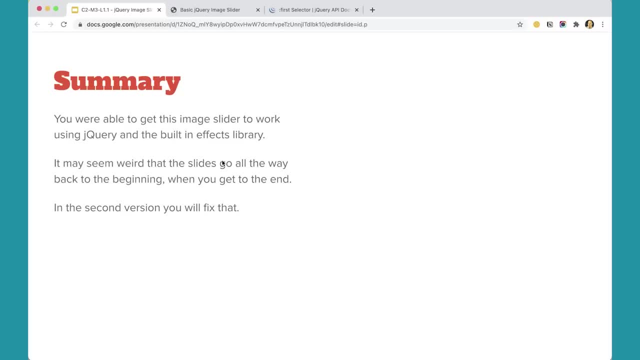 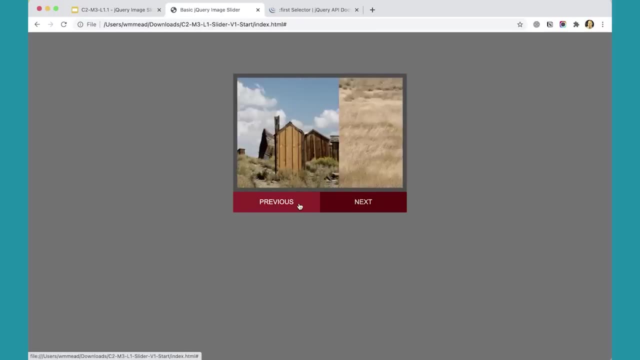 And that's really great. So we were able to get all of that to work. Now it might seem kind of weird that the images, when it gets to the beginning here, it sort of moves the whole strip over to the end. Wouldn't it be kind of nice if it kind of wrapped around instead? 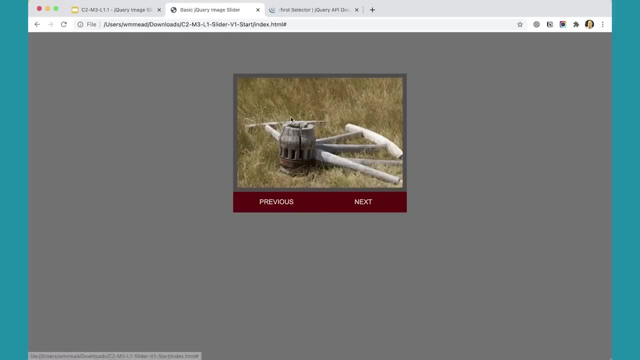 And that's what we're going to do in the next project. We're going to take this script and push it further so that we can actually make it so that it wraps all the way around. We'll take a look at that in the next project. 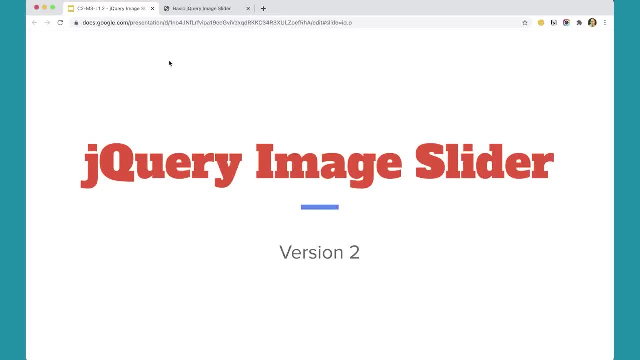 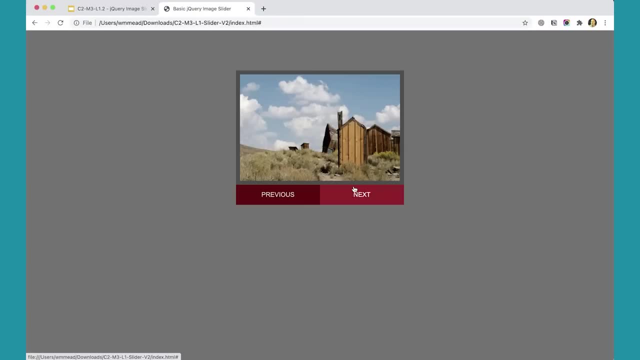 jQuery Image Slider Version 2.. In this version, we're going to take the slideshow that we already have, the slider that we have with the images sliding in, the one that goes to the end and then brings you back to the beginning and works as a strip. 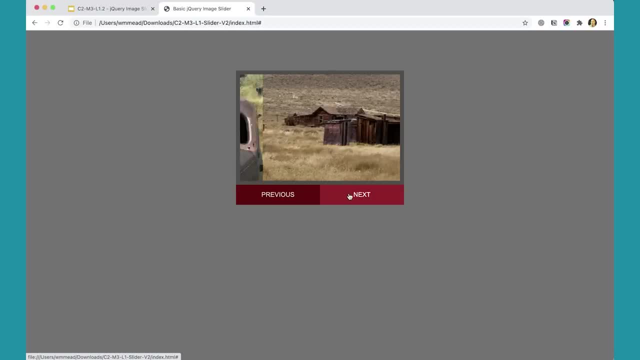 We're going to take this thing and make it so that it wraps around, so it feels a little bit more natural, And I think that will be kind of a nice effect if this thing wraps around like that. So we're going to take the same set of files that we've already worked on. 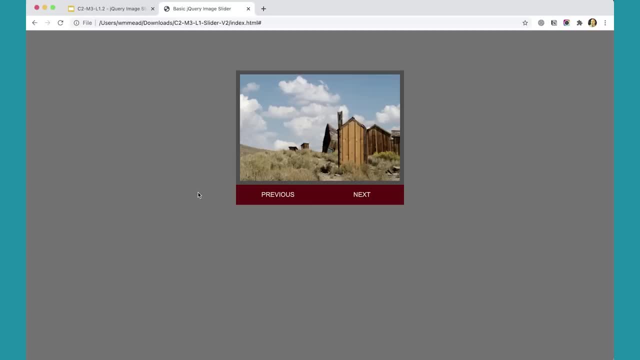 and we're going to rework them to create this next version of this slideshow. And, by the way, this is a really great way to learn. JavaScript is to make a small project and then look at it and go: you know, what could we, what could I do to make this a little bit better? 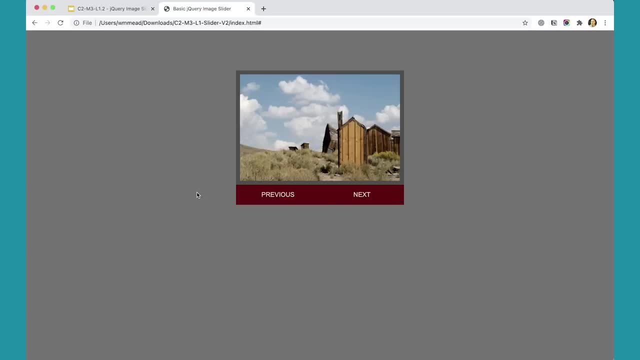 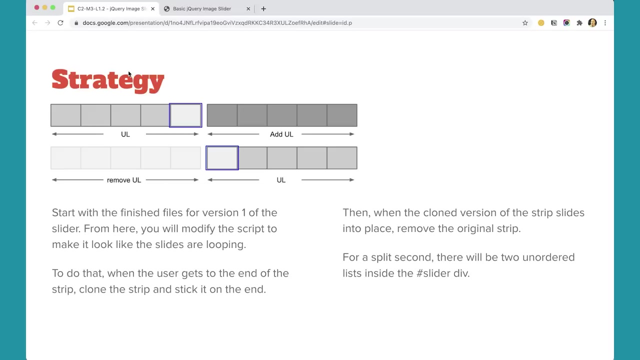 and work on ways of revising it to improve it and make it a little bit better. And this is a great way to learn JavaScript and a great way to challenge yourself, to take on new coding challenges and learn new things. So what's our basic strategy here? How is this going to work? 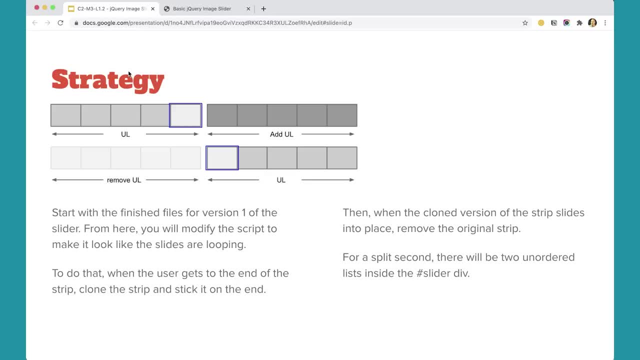 How are we going to make it wrap around? What we're going to do is we're going to basically clone the entire strip of slides so that if we look at this top picture here, if you click the next button all the way till you get to the last slide in the strip of slides. 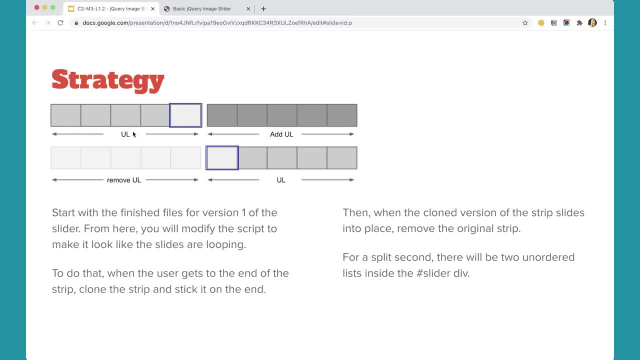 we're going to clone The entire unordered list, the UL, which is the unordered list with all the slides in it. We're going to clone it and tack it on the end so that when you click next again, this one slides into place and it's on the first slide. 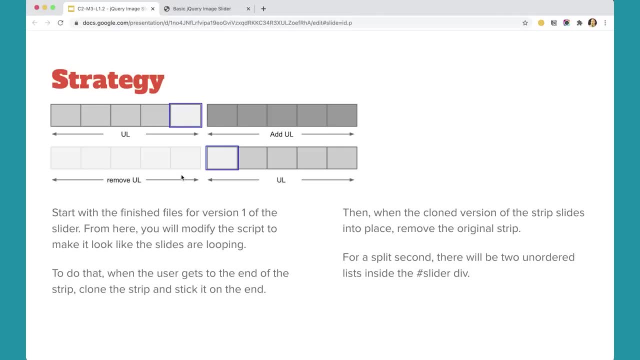 Then we can remove the one, remove the unordered list that was there before, and it will go away And we're right back where we started with a strip of slides on the first slide and we can keep going forward And then, if you click the reverse the previous button. 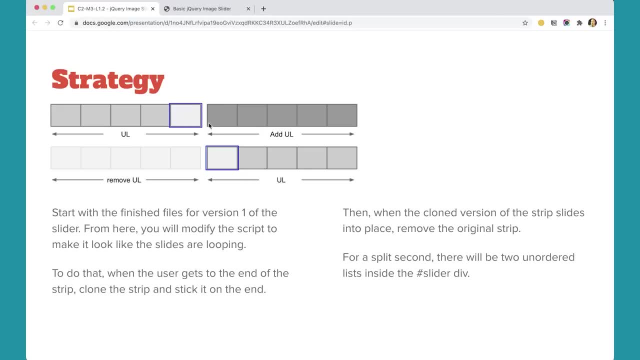 it's just going to do the same thing in reverse: Instead of tacking it on at the end here, it'll tack it on at the beginning. So that way we will always have kind of an unending loop of slides, whether you're going forward or backwards through the slides. 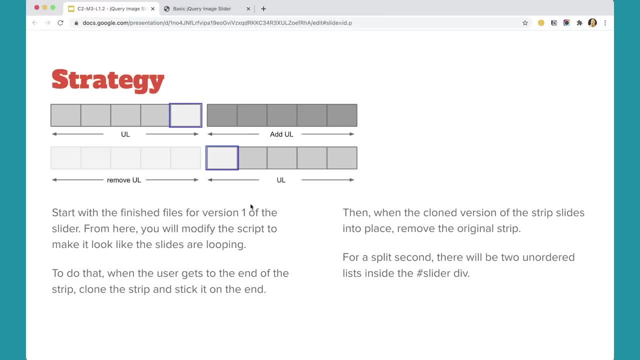 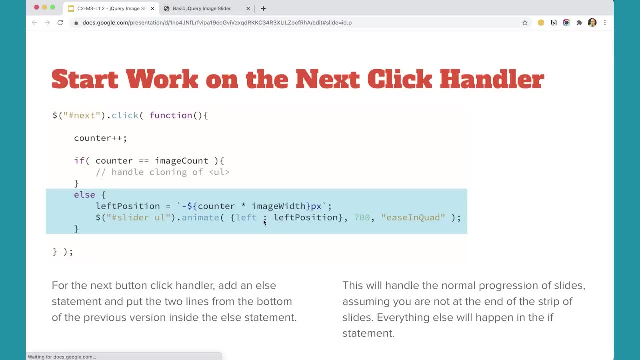 That's the basic strategy that we're going to use to make this thing work. So the first thing we can do is to start to work on the next click handler and make it different- a little bit different from what we had before. We're going to add an else statement in: 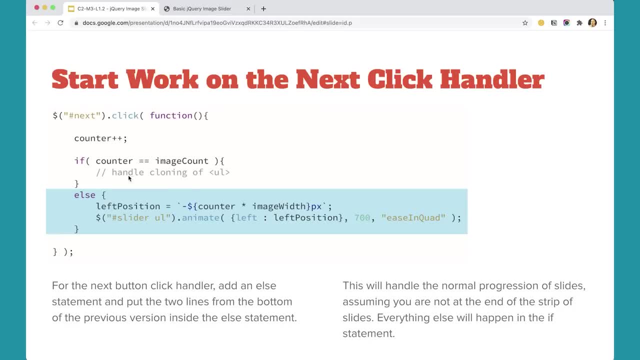 The if statement is going to handle the cloning of that unordered list and what happens when we get to the end, But the else is going to handle what happens if we're just on a slide in between, in which case we're just going to move forward in our in our slides. 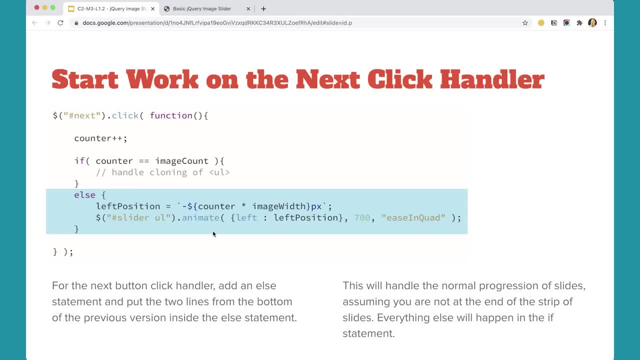 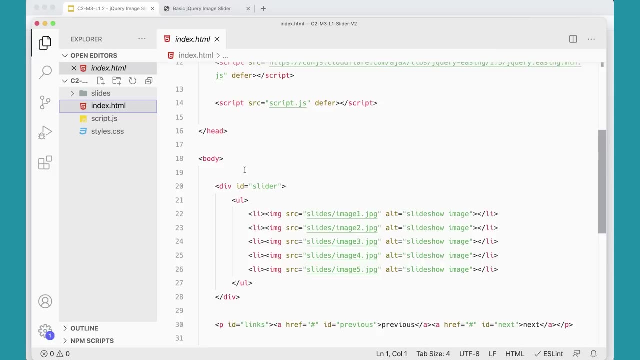 So this is the exact same code that we had before. We're just going to move it so that it's inside of an else statement. So let's go over to our files, And here I have nothing's really changed here. This is the exact same set of files that I had at the end of the previous script. 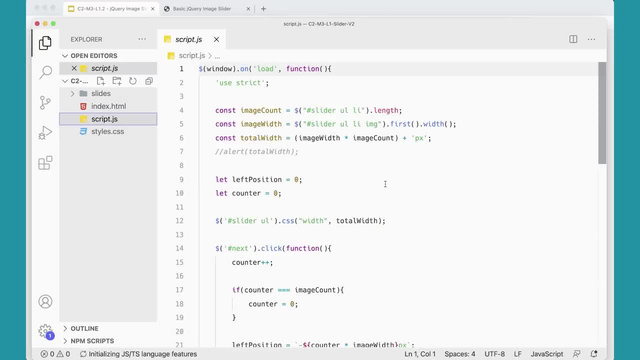 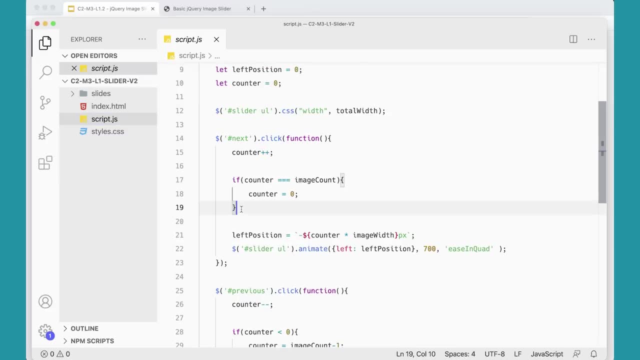 the previous version of this slider, And in here I'm going to just come down to my my next click handler. I'm going to add an else in here, Else like that, I'm going to move this stuff Into the else. 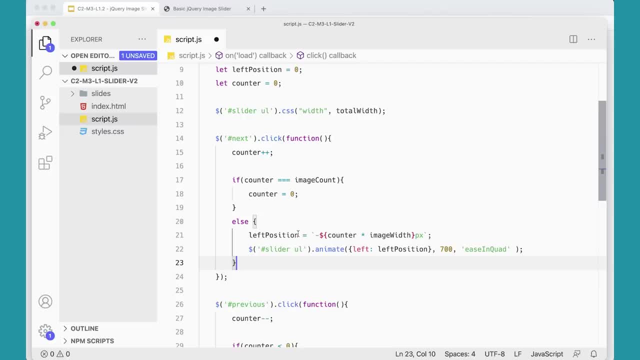 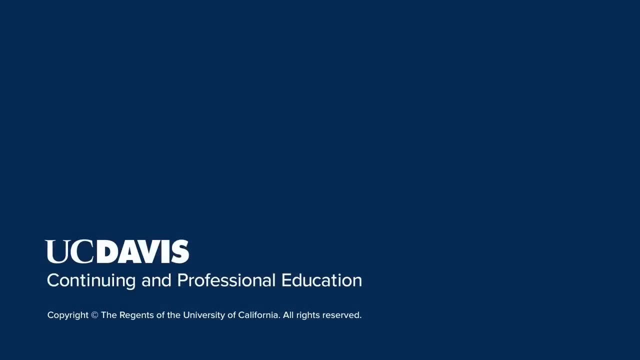 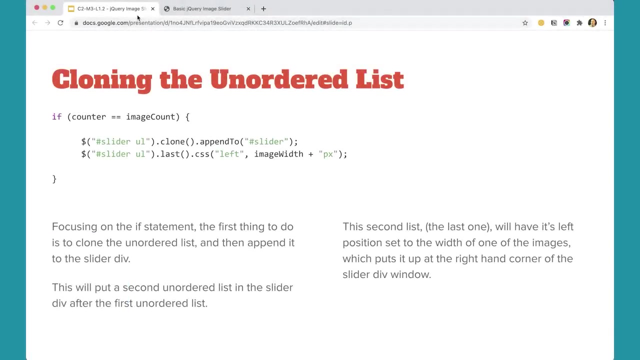 We're going to do something very different here, And we'll take a look at what's next in the next video. The next thing we're going to do is we're going to clone the unordered list using the jQuery clone method. You can see, here we've got a clone method. 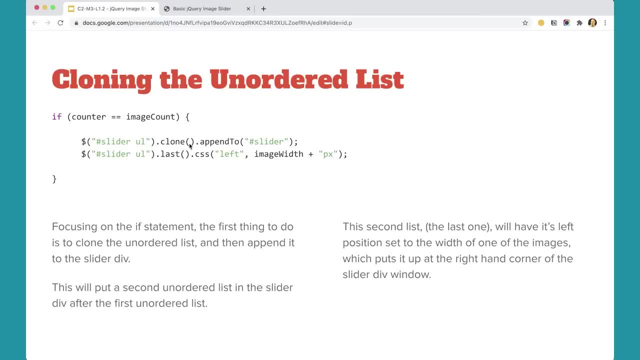 that will allow us to take that entire unordered list and make a clone of it And then we're going to append it to the slider. That'll put it at the end of the element Of the element slider. So what that'll do if we come over and look at our code here. 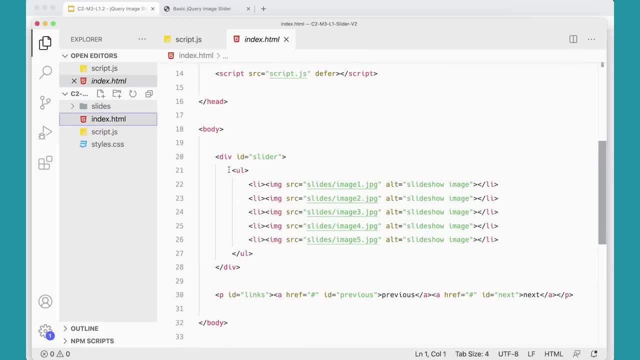 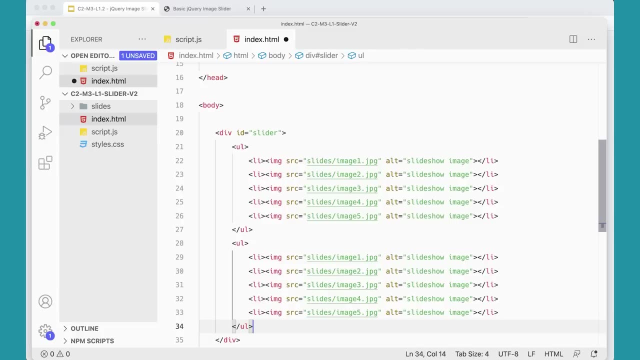 if I look at my index here is: it'll take this entire unordered list and make a copy of it and stick it right here Like that. It's going to end up looking like that when it's done. When it's done cloning and appending. 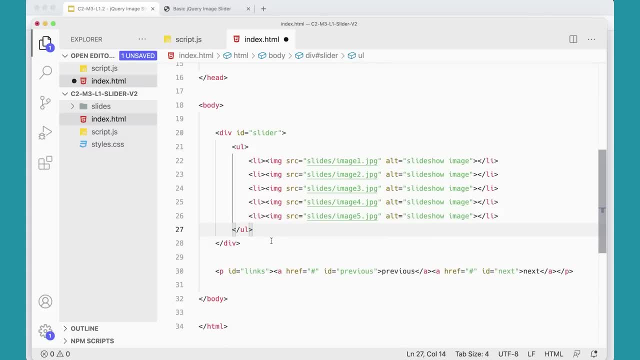 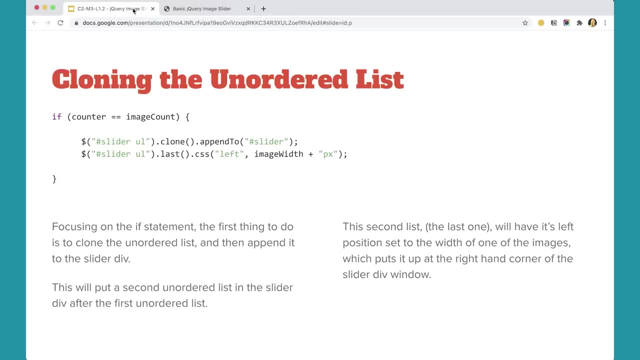 That's what it's going to do, Sort of in code, Rather than physically adding the HTML like I just did there. So it's going to add that on there, It's going to clone it And then append it to the slider. 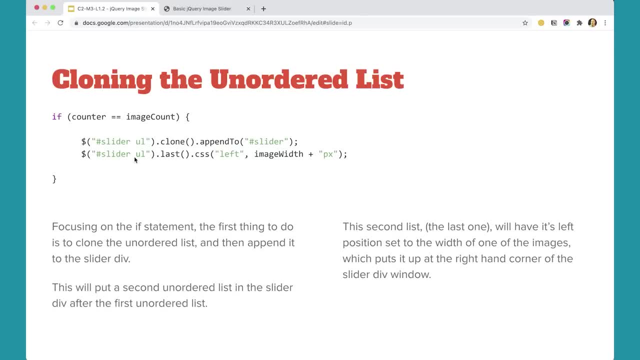 And then I need to set the CSS of that second unordered list, The last one. I'm going to set the left to image width plus pixels. So it's going to be positioned right here, Because this is our little window. So it's going to say okay. 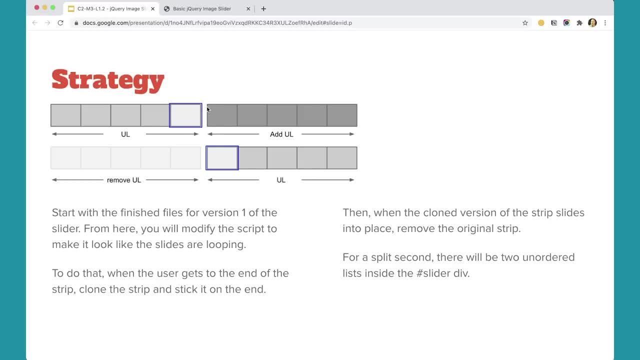 left. since the image is 400 pixels wide, it's going to set the left at 400 pixels. That'll put the corner, the left corner, right up against the edge here, Which is exactly where we want it to be. So that's what's going to happen here as we work on this. 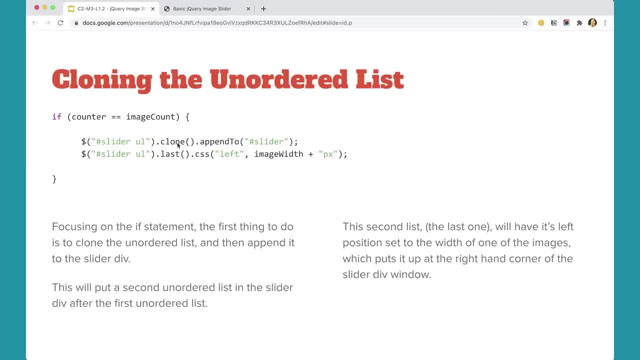 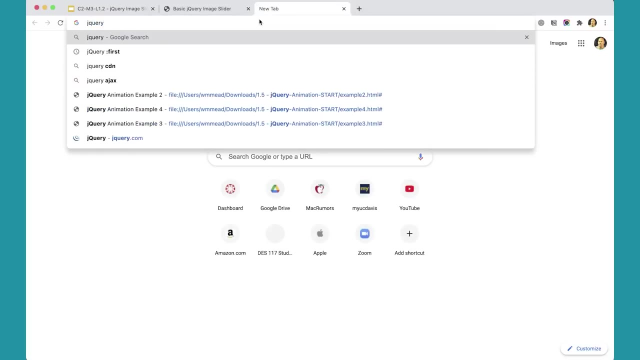 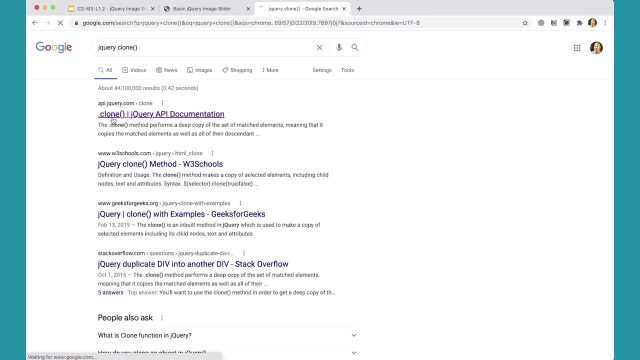 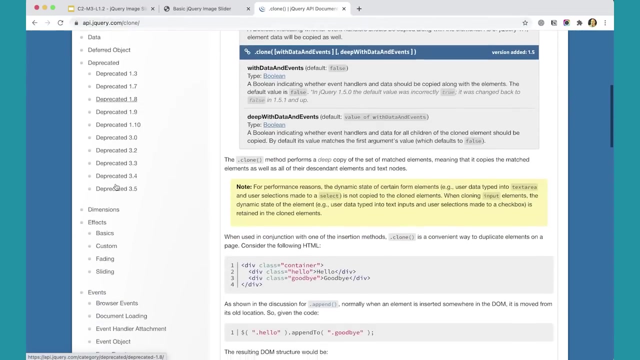 and make this go here. Also, you might be wondering: how would I know about clone or something like that? You can go to the jQuery documentation really easily: jQuery clone And the apijquerycom has all the documentation for all the different things that you can use with jQuery. 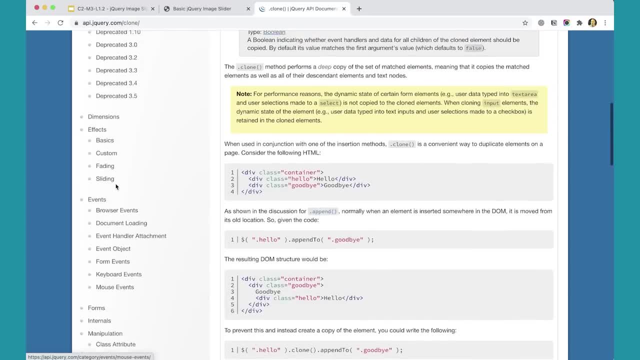 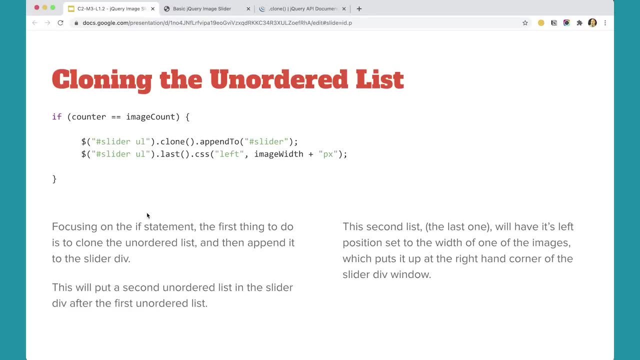 And it's really just a matter of looking through and seeing what the different functions are and what they do and looking them up. It's kind of fun to pour through the documentation sometimes and see the different examples of things that you can do. So that's the way that would work. 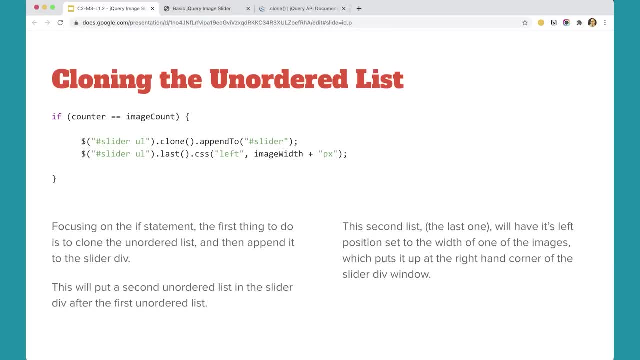 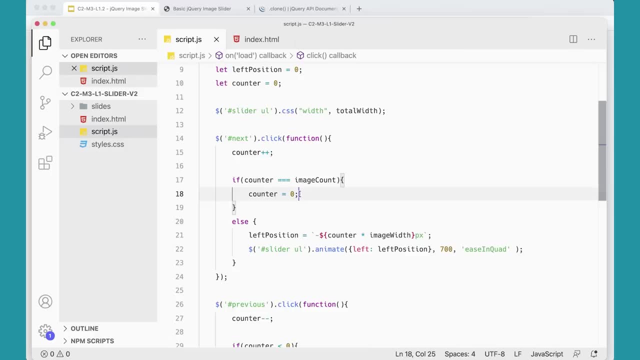 Okay, let's go ahead and add this to our script. So I'm going to go back to my script file here And you can leave the counter in if you want. All this stuff is going to come before the counter. We're going to do the counter thing at the very end. 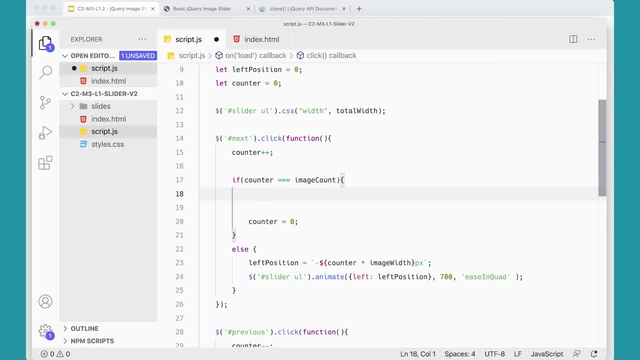 So you can leave the counter in if you want, or you can take it out and put it back in at the end. It doesn't really matter. But I'm going to use my jQuery object To go get pound slider and get the ul. 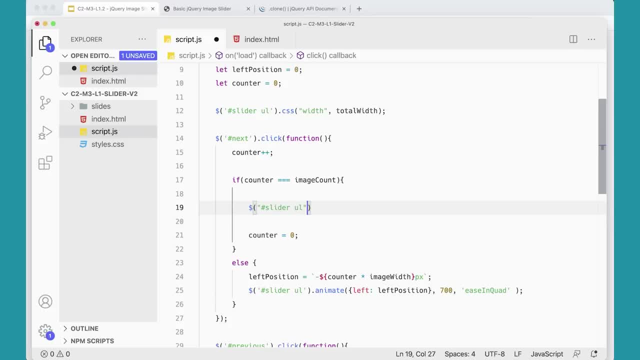 the pound slider unordered list And then I'm going to clone, it clone And that will make a clone of that unordered list And then I need to append that clone to slider. pound slider clone. Don't forget the pound sign. 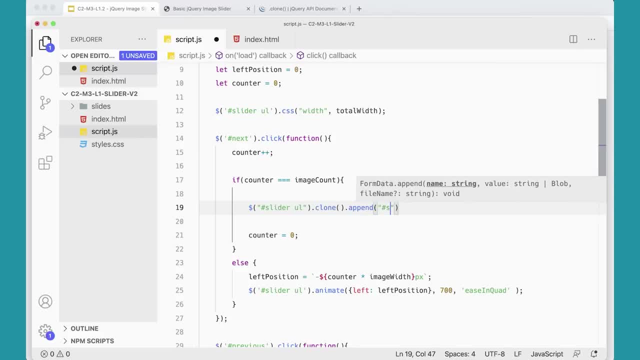 Append it to pound slider And that will actually make, when we get to the last slide, that will make a clone of it and put it on there, And then I need to set the position for that one. So I'm going to say again: I'm going to get my jQuery object. 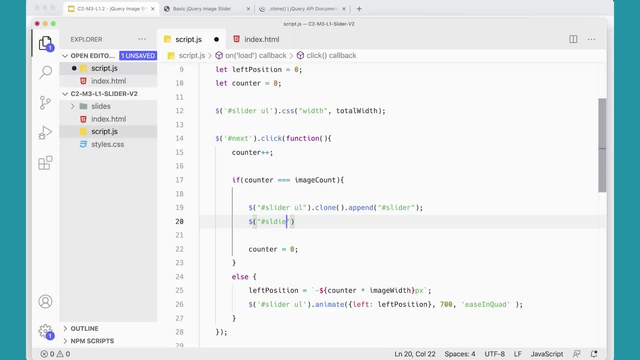 pound slider ul clone, But I want to get the last one. Now I have two, So I want to get last. We're going to use this last method again. I'm going to get the last one and I'm going to set it to CSS. 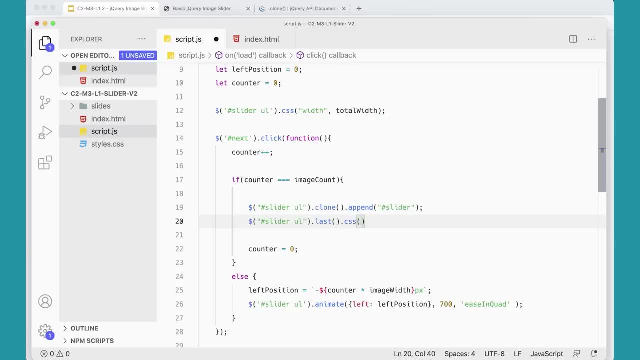 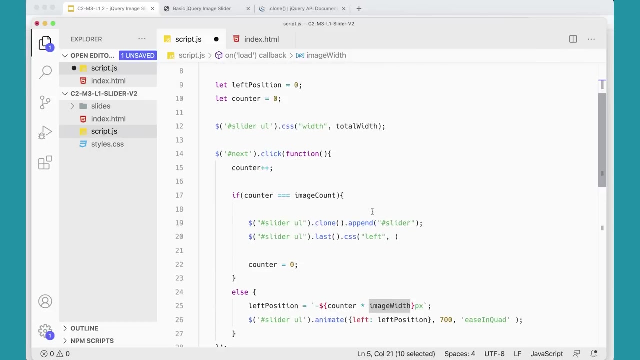 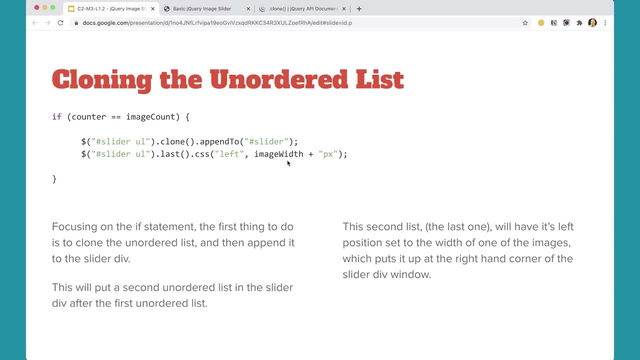 And I'm going to set the left position left. And what am I going to set it to? I'm going to set it to image width: Image width plus- I probably need pixels on there right. Image width plus px right. 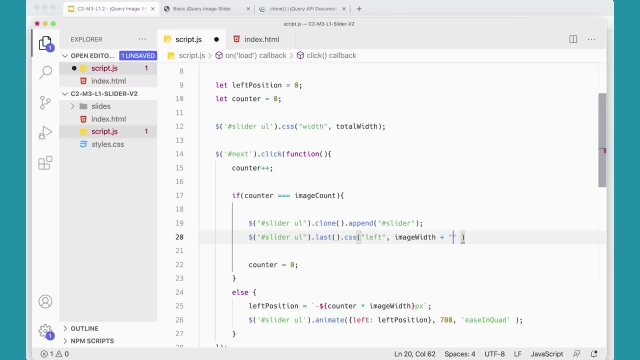 Image width plus quote px, And that will put it in exactly the correct spot here on the page. That will put it so it shows up at the end. Okay, so now it's shown up on the end, And in the next video we'll actually handle the animation. 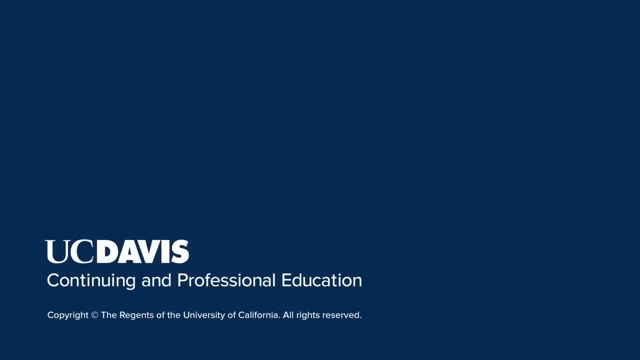 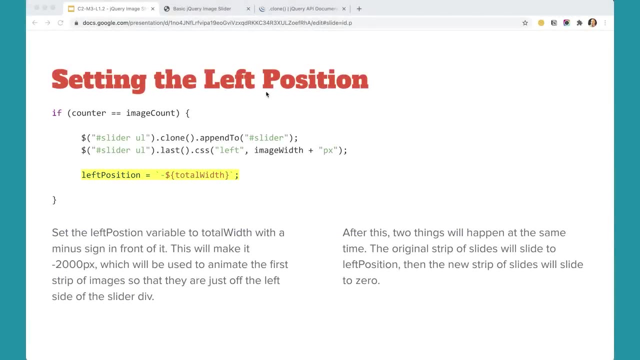 Before I do the animation, I want to set the variable left position equal to a value where I'm going to move that first unordered list to. And in this case the unordered list is 2,000 pixels wide. That's total width, because the images are 400 pixels each. 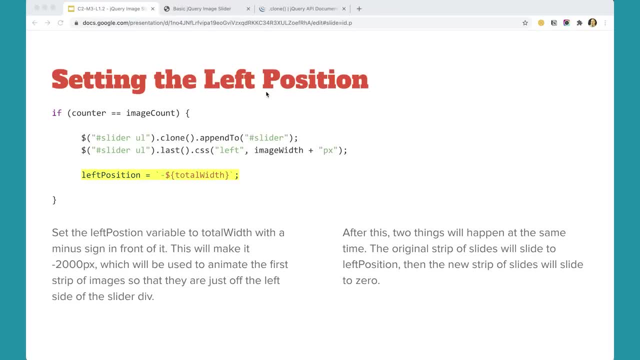 and there's five of them. so that's 2,000 pixels. So I'm going to move the left position to minus 2,000 pixels. What that'll do is it'll move that entire first unordered list where it sets the correct position for that first unordered list. 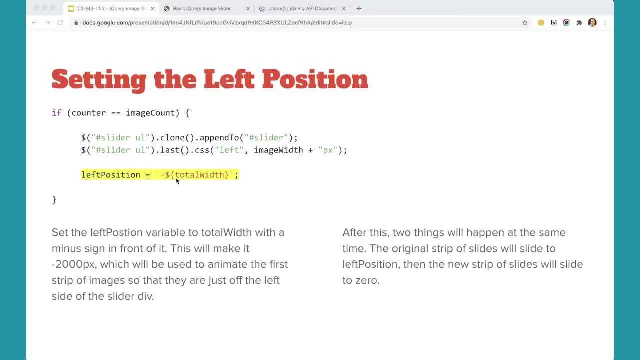 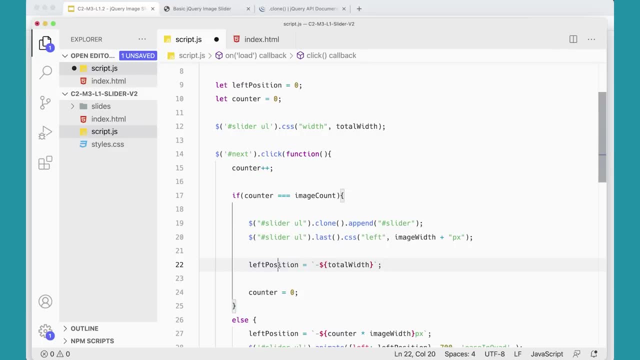 so that it's entirely off the left side of my slider window. So let's go ahead and do that. first, I'm going to put in left position equals and then use my tick marks and a negative sign because it's going to be minus. 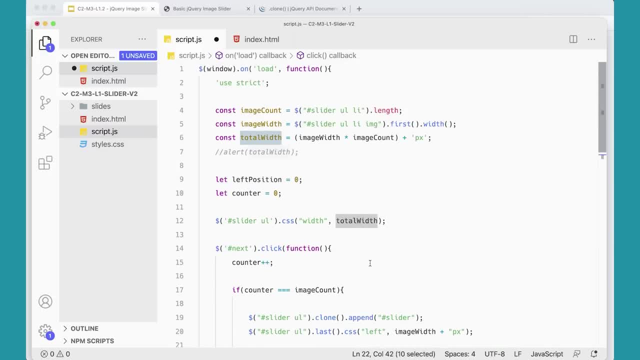 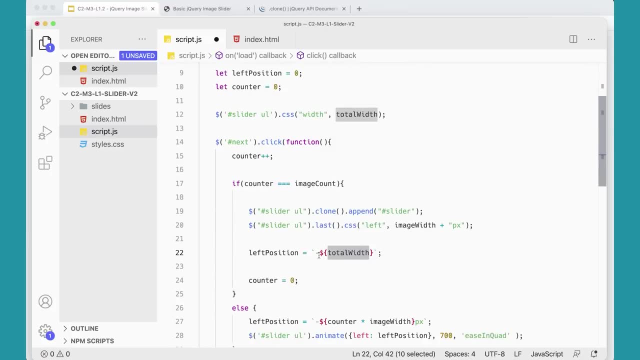 and then total width is going to evaluate to 2,000 pixels because, remember, total width is the image width times the image count plus px. So that's going to say minus 2,000 pixels. right there, Great. So that puts that into the correct place. 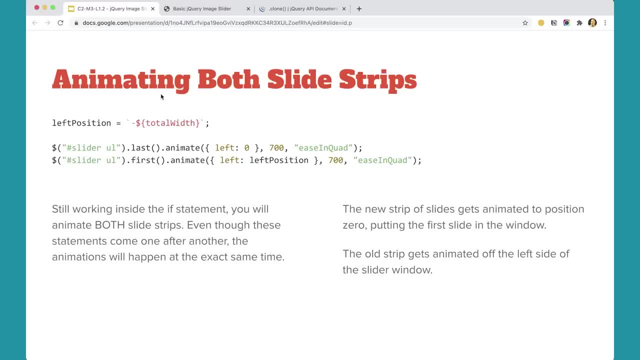 Okay, so we've got that variable set. Now what we need to do is animate both unordered lists. I'm going to animate the first one and the last one, And they're going to animate at the same time, so they both move at once, at the same speed, into the correct positions. 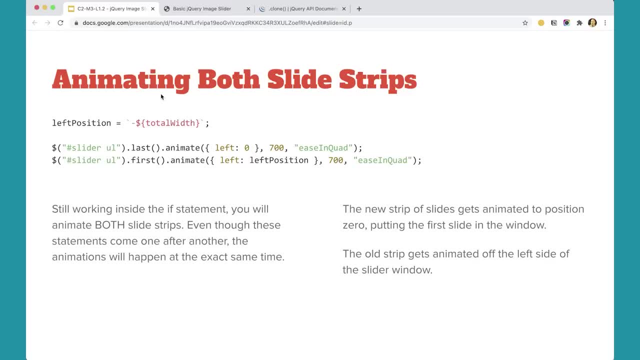 In this list I'm moving. the first line moves the second unordered list, the last one, the one that we added with our clone, our cloned unordered list, And it's going to move that to left zero, so that it's moving it from the left side of that window. 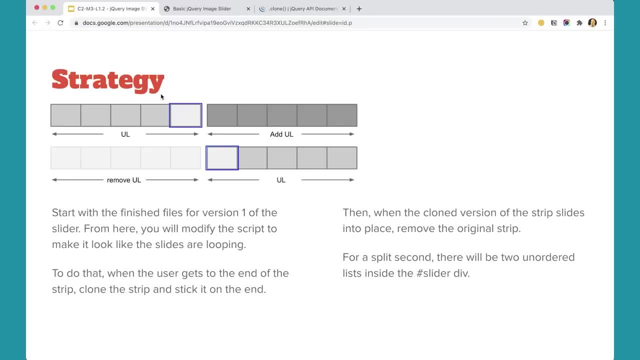 We come back up here to here. It's moving it from this left corner of the window into its space here, So that's going to put that into the correct place, Whereas the second one is going to move from this space all the way out. 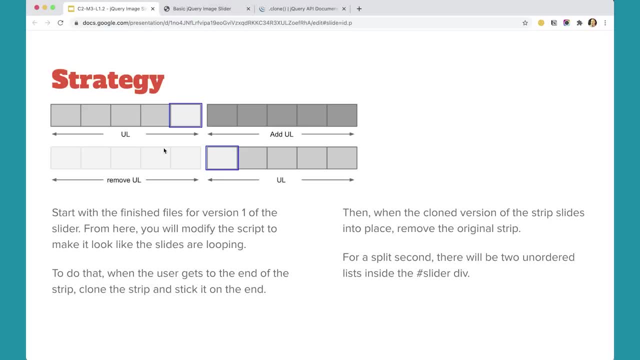 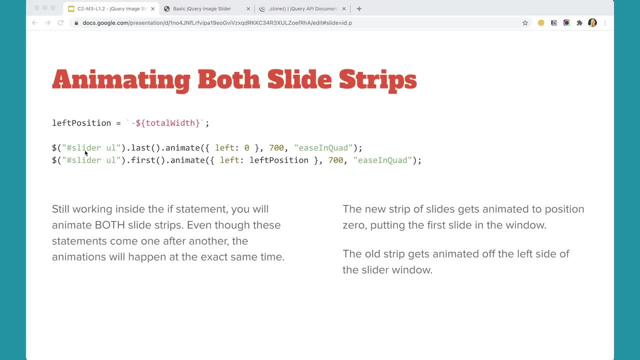 so that this point is at minus 2,000 pixels, which will put this edge right, at this edge here. So you can see, here I'm getting slider ul, last the last one animating it. I'm animating the left property to zero. 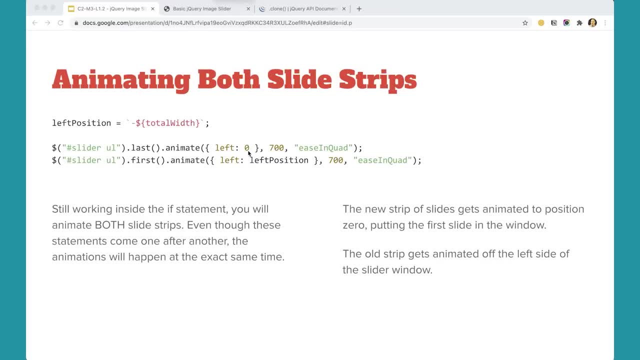 So that will put it right, so that the first image is right in position inside my slider at 700 using ease in quad, Whereas the first one gets animated to left, left position, And we just set that to minus 2,000 pixels, also at the same speed. 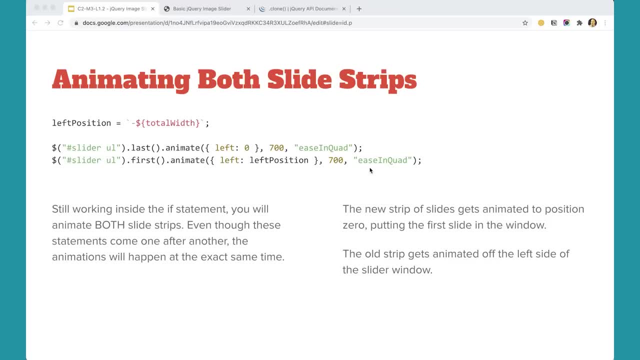 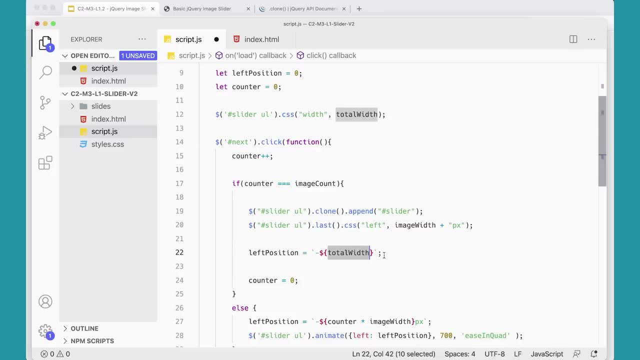 using the same easing so that they kind of move together. So let's go ahead and add this into our script over here. So I'm going to say: get my, get my pound slider, oops, quote: pound slider ul. 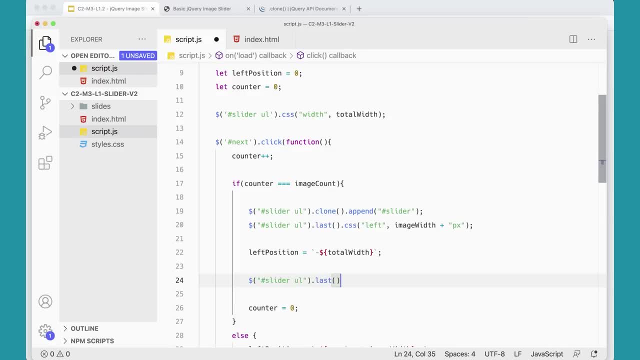 dot last this one, And I'm going to animate. I'm going to animate it. How am I going to animate it? I'm going to animate the left property to, uh, zero. That one goes to zero. Left goes to zero. 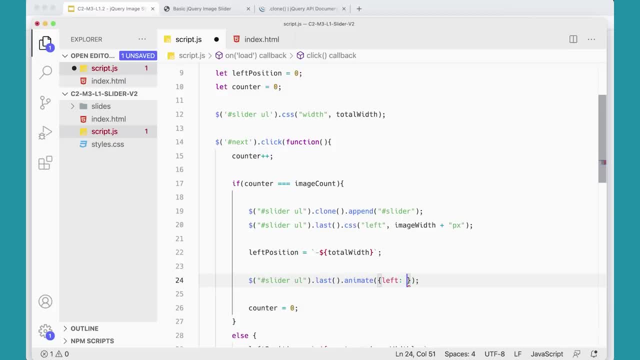 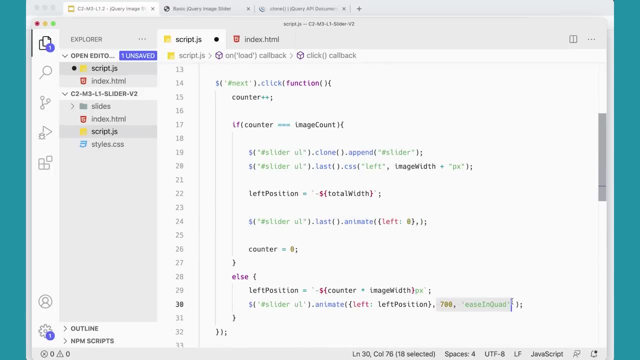 And I'm going to just use the same easing and everything else that I had down here. I can even just copy and paste that to move that into place. So that moves that one. I can copy this line and paste it here, But now I'm going to move the first one. 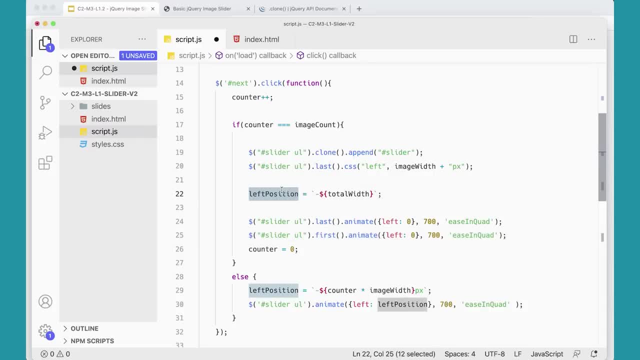 animate left and it's going to get moved to left position. There we go, So that will move both strips at the same time. It's going to animate them into the correct place. Then the last thing that we need to do is remove this one. 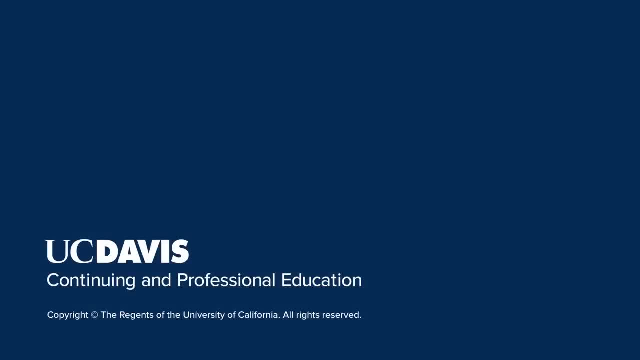 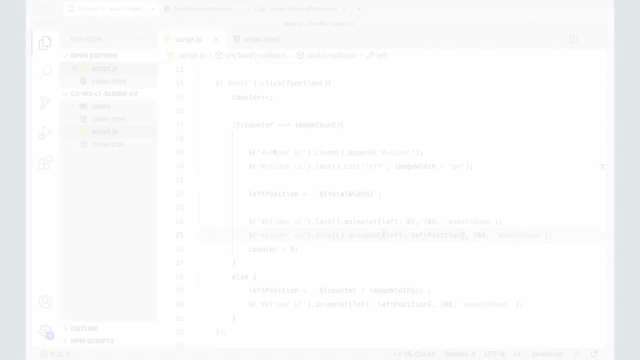 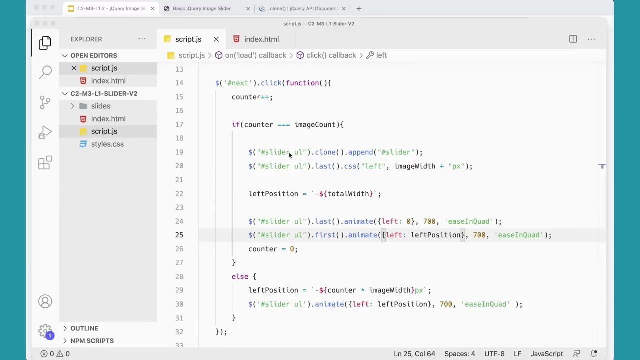 And we'll look at that in the next video. So far in our next click handler, we've checked to see if the counter equals the image count. If it does, we have cloned the unordered list and then added it to our slider. 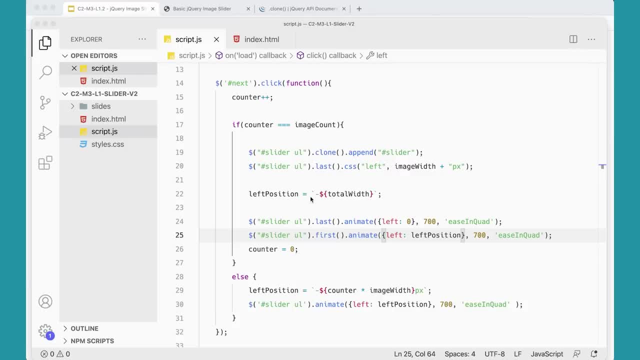 and then set its position into the correct place. Then we animated the two unordered lists at the same time, the first one and the last one. We animated the last one so that its left position puts it right, so that the first picture is inside the window. 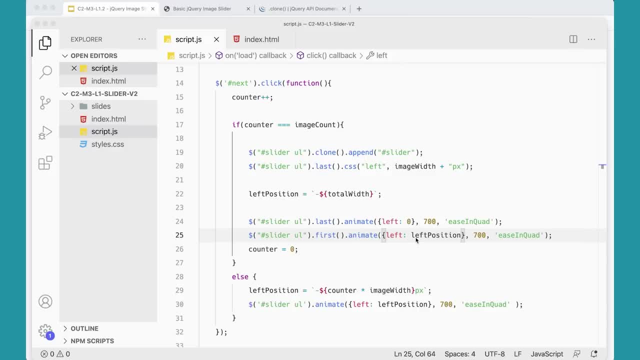 and we animated the first one off the window, So that's the left side of the slider. Then the last thing we need to do is, after this animation is completed, I want to remove it from the DOM altogether. So the key word there is: 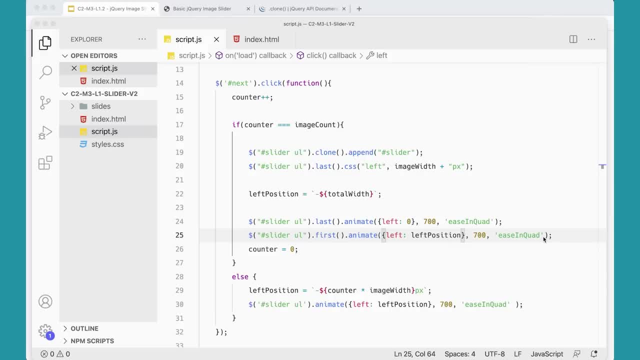 after this animation is completed. So that means I need a callback function. So in here, after the ease in quad, you're going to put a comma and add a function like so And it's wrapping around funny. I'm going to close this explorer here so you can see it better. 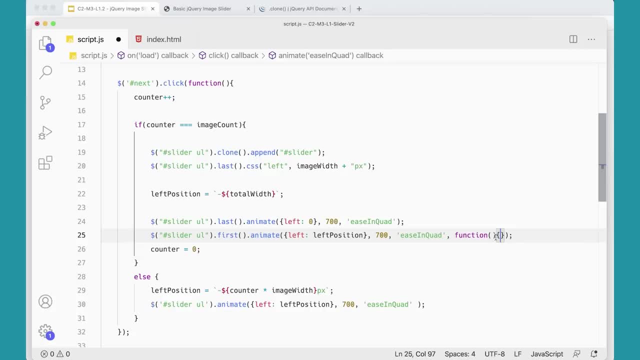 But this function is a callback function that runs when this animation has completed, And that's what I want to do here. So I'm going to click inside of there and move that down And then I can say I want to actually remove this first one. 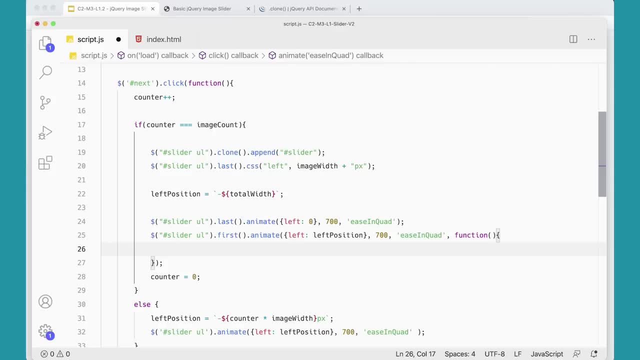 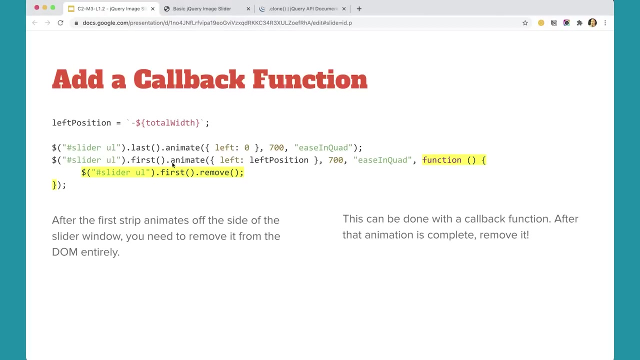 So I can say dollar sign, get my jQuery object And say here pound slider, ul, dot. first the first one, dot remove, And that will take it off the DOM entirely. So you can see here on my slide that's what I have here. 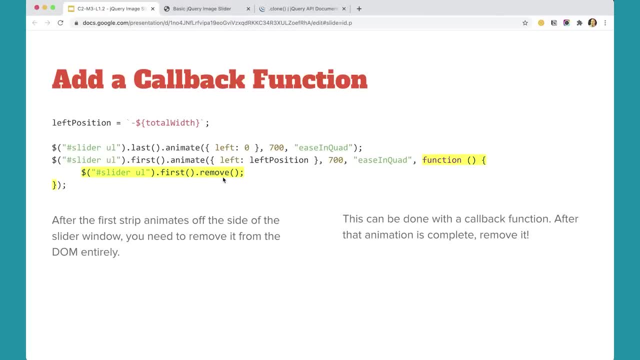 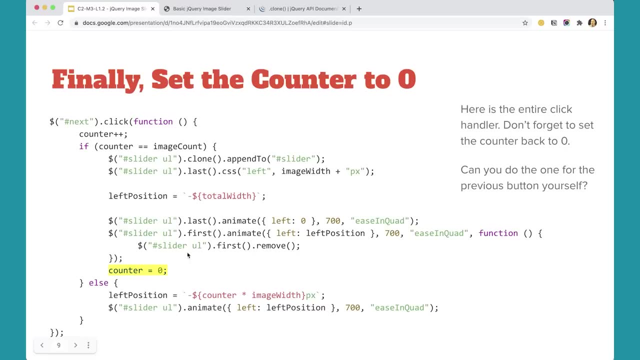 Pound slider first remove, So that will take it off, And then, once that's done, and then, once that's off, I can set my counter to zero and everything's back where it should be. So make sure you have down here: counter equals zero. 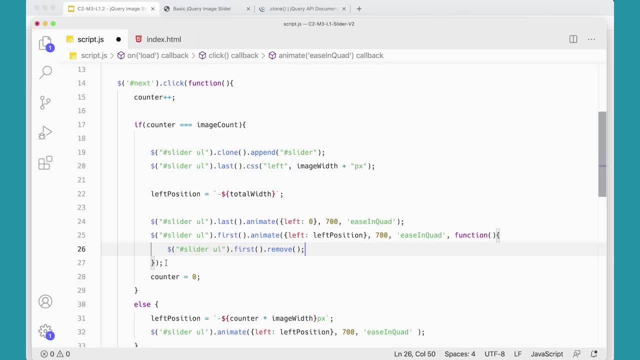 If you took it off before, make sure it's there now. Okay, So we've got that in place. We can even put a space there and make it so it's nice and clear what's going on. You could add some comments if you need to. 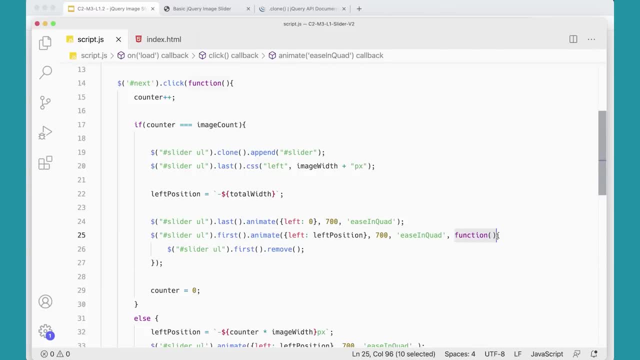 Sometimes it helps Make sure this thing is running as a callback function And that these two are running at the same time. And then, moment of truth, we get to test it and see if this script is actually working properly. for the next button. 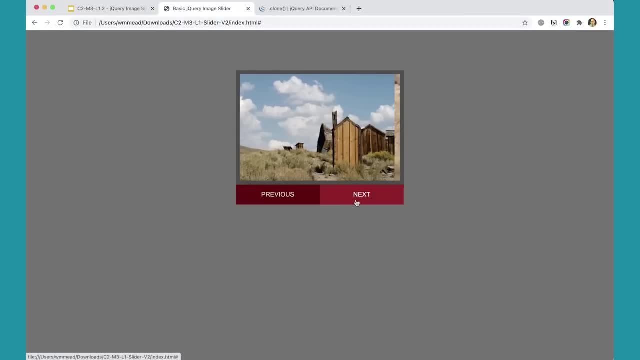 Click refresh. When I click next, next, next, next, Now it should, without wrapping. it should wrap around and put the next one in. Let's see if it did it right. Whoops, something went haywire. Let's see what we did wrong. 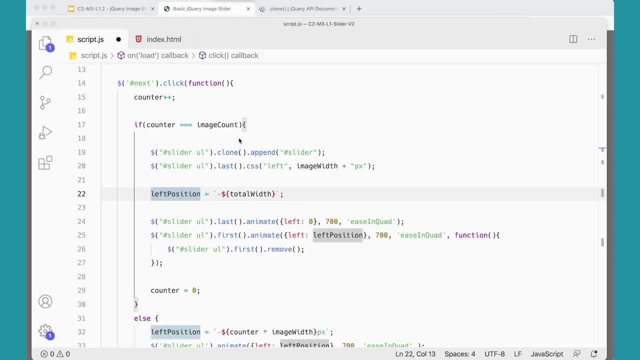 Let's see if we can figure this out, because it's very common to make a mistake in your code like this, And it's important to be able to develop the skills to troubleshoot and figure out what's going on with it, And this is a really good example. 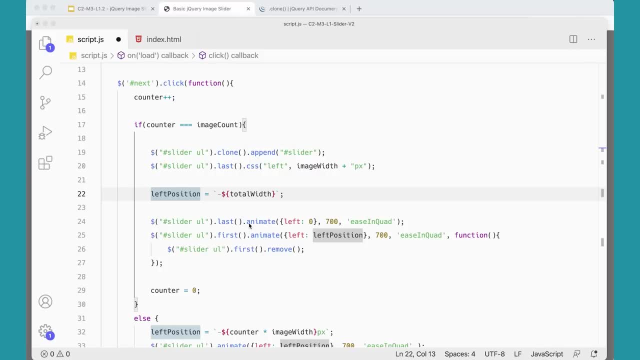 of something that can go terribly wrong, because you can tell the script is not working properly at all. So I'm looking at my script and it looks like. I look at it and logically it seems like it's set up right. So I must have some sort of error in here somewhere. 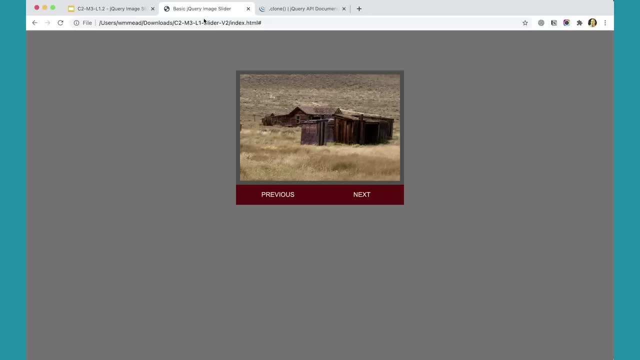 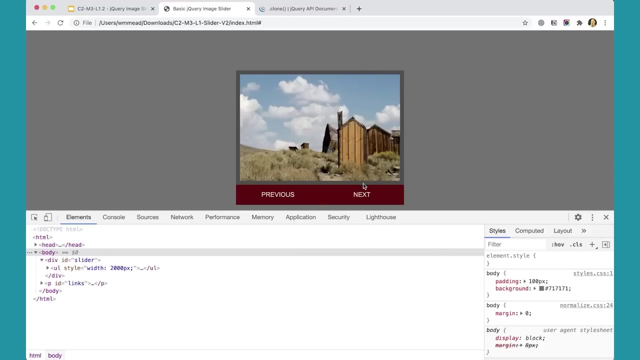 So the way to solve this problem is to come back here and refresh the page and then inspect And use the inspector and see if you can see what's going on. So if I come down here and look at my slider and I go to next, 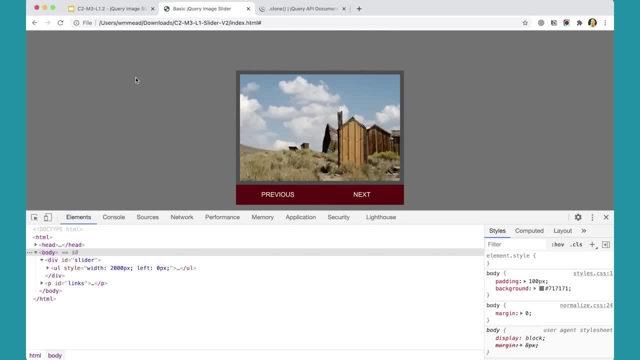 when I get to the end. something weird was going on here, Right? I don't know if it's working right, But let me make sure everything is saved properly over here. Save this, Come back, Refresh And let's just see. 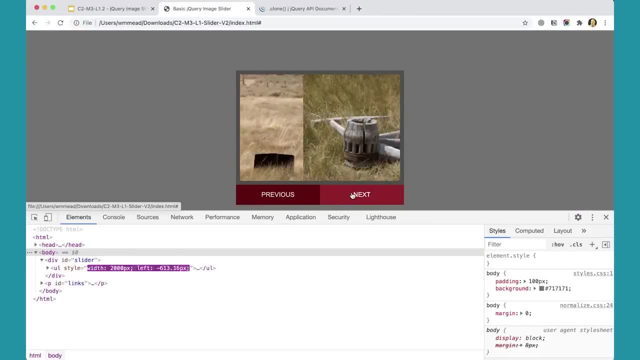 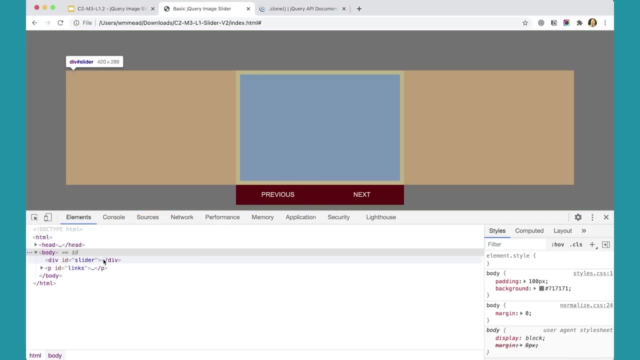 So if I look at my slider here when I get to the end like something is going really haywire there, What's going on? I look over here and my slider doesn't have any unordered list in it at all. What the heck is up with that. 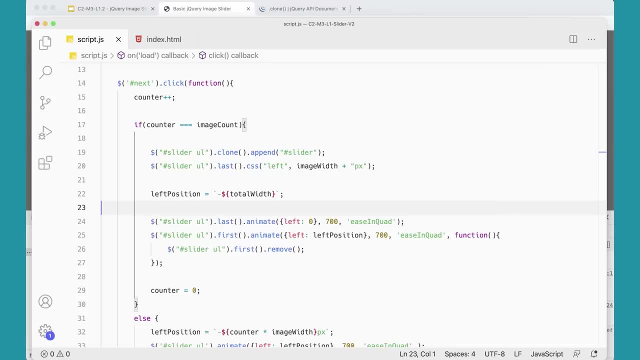 So the way to solve this, the way I go about solving this, is to come back here and start by commenting this out. I'm going to just comment this out and see: is this part of the script working? Is it cloning and doing what it's supposed to do properly here? 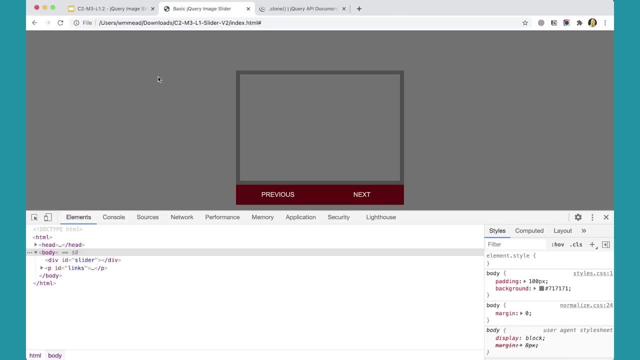 So I'm going to just do that And I'm going to come over and refresh, Refresh And watch my HTML here Because, remember, JavaScript is just manipulating the HTML, So let's see what happens here. That goes And it goes. 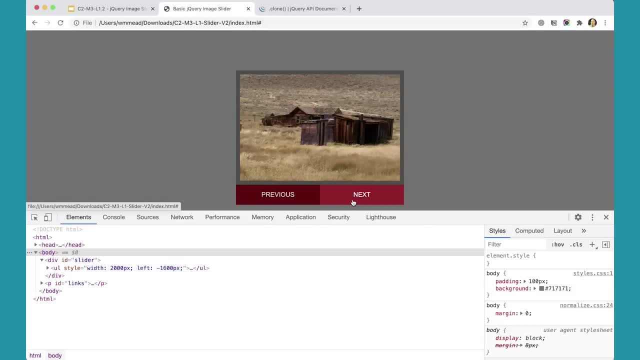 And it goes, And it goes When I get to the last one it's not cloning properly. It's not cloning my thing properly, So something's wrong with my line with the cloning. So if I come back and look at this, 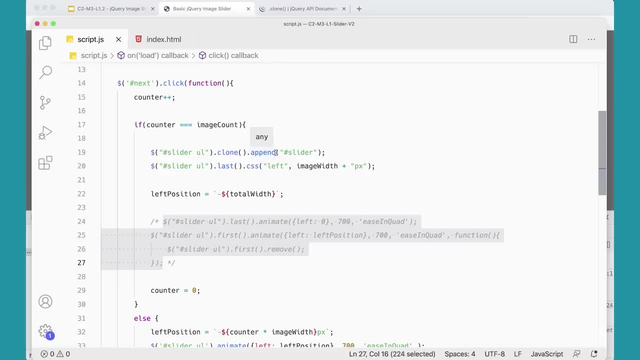 I'm like, oh, append. This should be append to. I'm using the wrong method here. That should be append to, And you may have caught that if you were looking at my slide carefully and thought, oh boy, you made a mistake there. 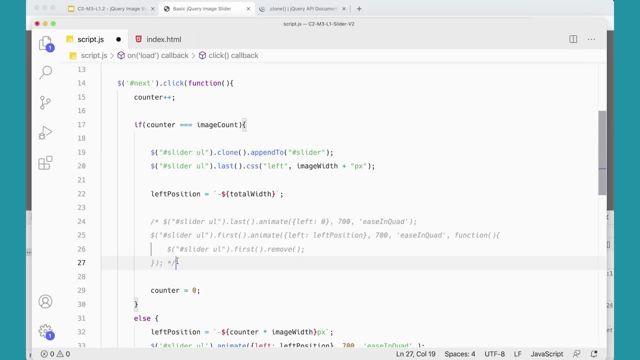 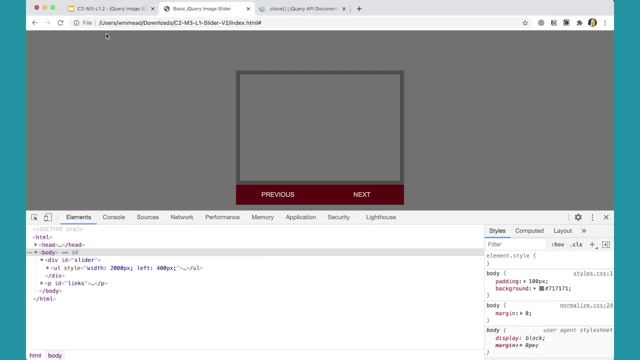 Maybe you even caught that before I did, So that should be append to. So it wasn't cloning properly, So it wasn't getting added properly. So then none of this was working right. So let's turn that back on and see if that solves the problem. 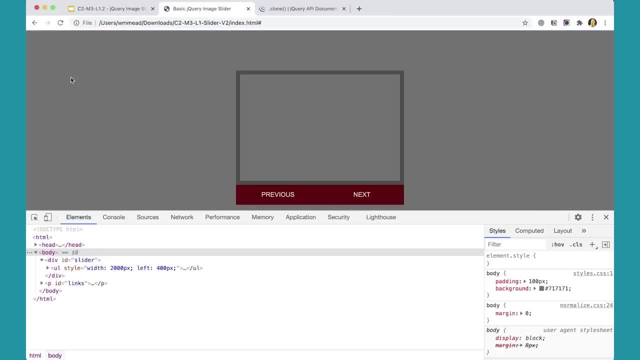 Come back here. But the inspector is your friend. It'll really help you solve these types of problems because you'll be able to sort of watch here and see what's going on: Next, Next, Next, Next, And then now, when I click next, again. 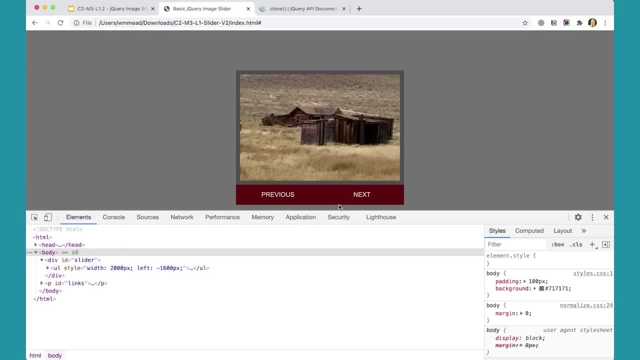 you'll see it should add an unordered list and then remove one. It'll add one and then it removes it. So it adds one on to the end, animates into place and then removes the first one. And now we're back to the beginning. 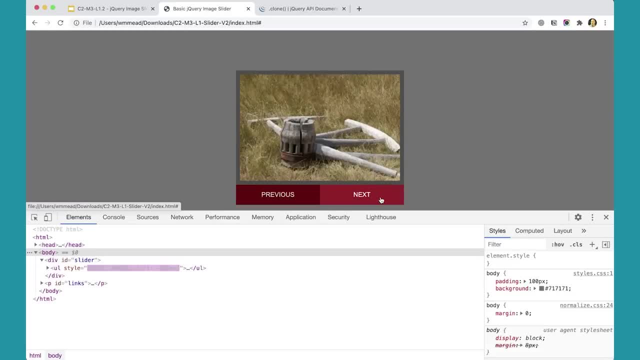 And I should be able to move through this very easily each time, And each time when you get to the end, it very quickly adds an unordered list and then removes one. So that's really cool. All right, great, So we're able to get that to work. 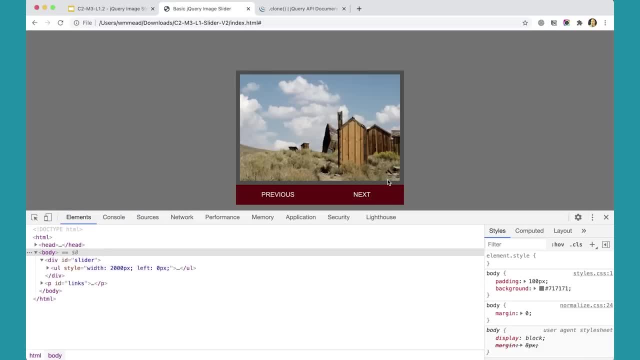 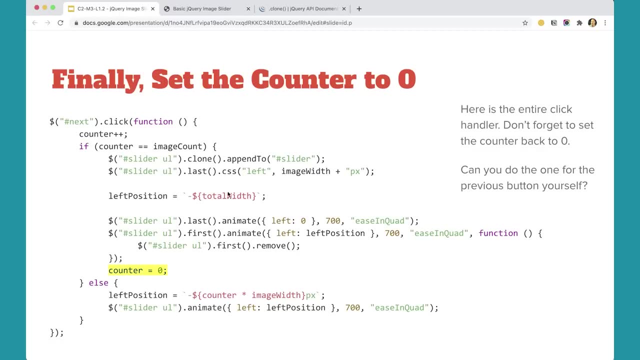 And not without any problems. but that's pretty typical in part for the course, And it's great when you see me make those kinds of mistakes, because I will make them and you'll make them too. Don't feel badly about it. But now the question is: 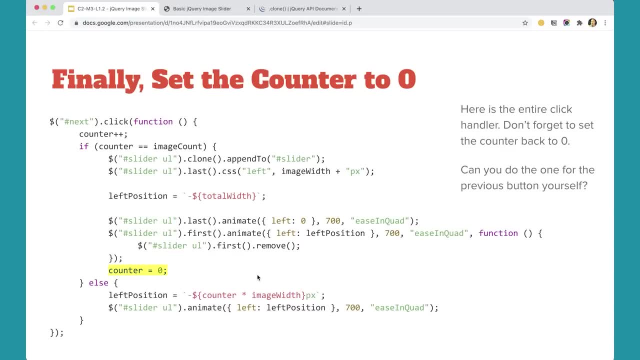 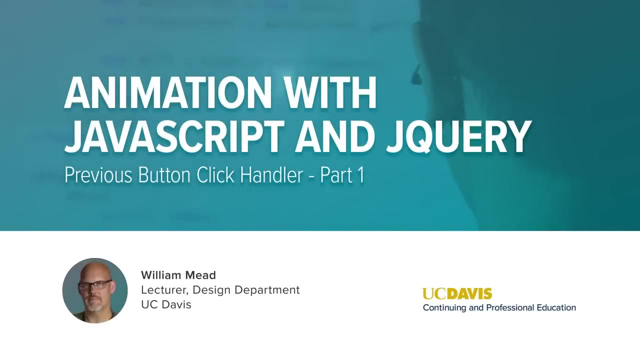 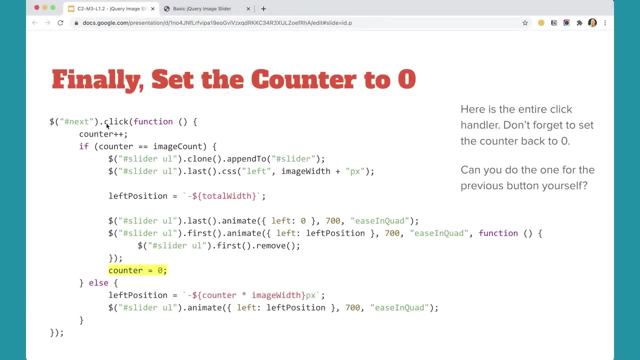 can you do the previous button link yourself? See if you can do that one, Try it on your own And then, when we come back, you'll see my solution for it in the next video. In the last video we figured out how to get the next click handler. 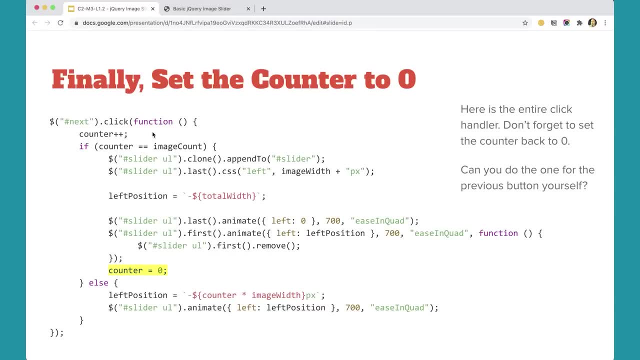 to function properly. We ran into a few problems, but that's pretty normal And we managed to fix them and we got it working. So now we want to get the previous click handler to work And hopefully you tried to do that and were able to do that on your own. 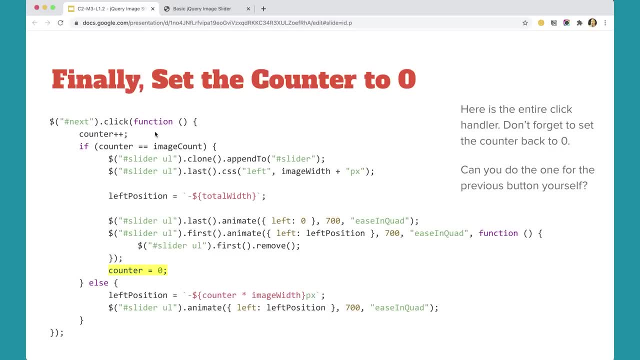 And if you weren't, don't feel bad. It's not easy. This is a tough problem because you have to really understand this stuff and think about it the right way. So let's do it together and sort of see how it's actually going to work. 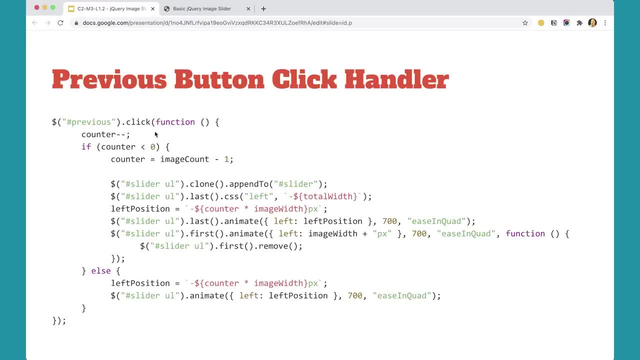 So the script I came up with looks like this. What's going to happen here is, when you click the previous link, the counter is going to get decremented, And then we're going to check to see if the counter is less than zero. 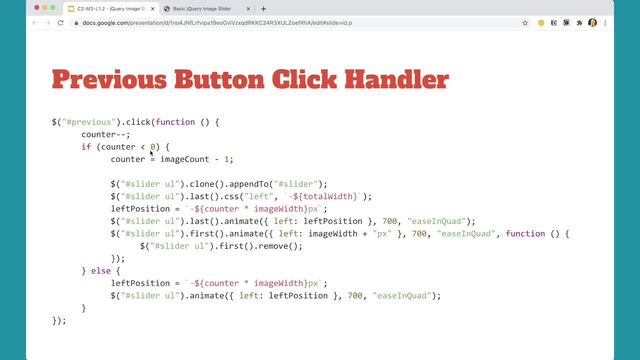 which means we've run through all of our images. So that's the same as before. And then we're going to set the counter to image count minus one. So we've got five images, And so we're going to set the counter back to four. 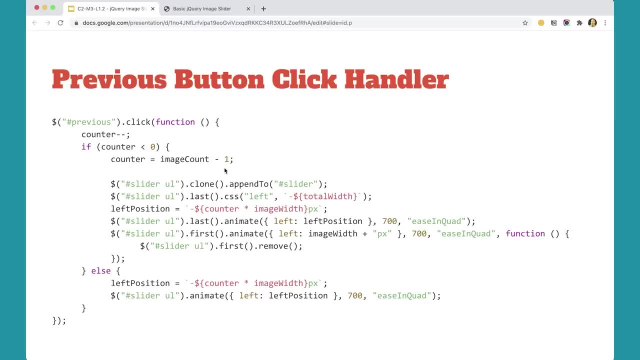 Remember our counter is always going to be a zero, a one, a two, a three or a four, Any of those five values. So we set it to image count minus one. So it's now a four. Then we're going to clone our unordered list. 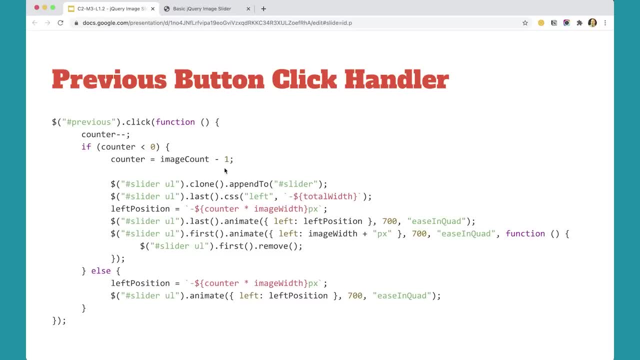 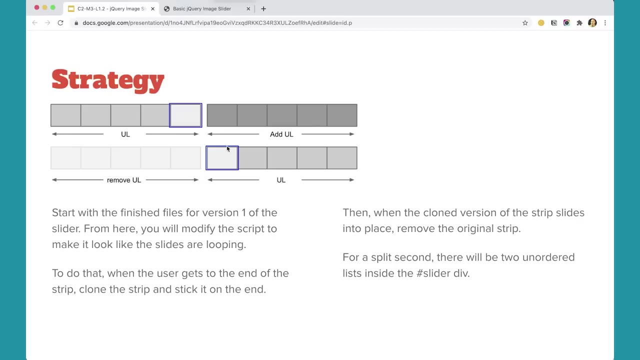 and append it to the slider, just like we did before. But here it will be helpful to go back and look at our diagram once again. Looking at our diagram, this is our situation in this part down here. Our strip is at this position. 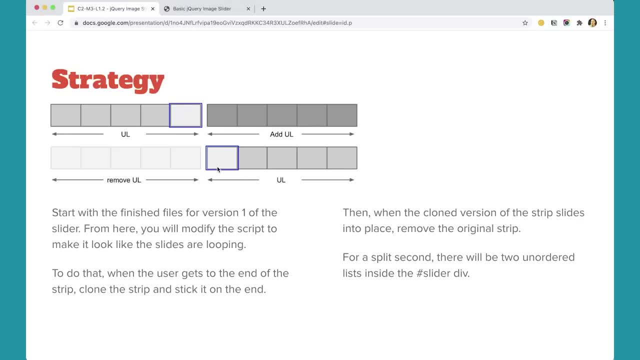 And we've clicked the previous button. What we want to do is we want to add the new strip and append it on this side. Instead of appending it on that side, we want to append it on this side of our slider And when you click the previous button. 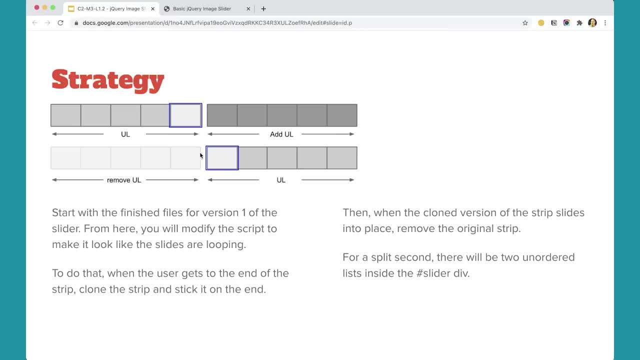 this one is going to move in from this position here And really we're tracking this corner here. So this corner is going to go from minus 2,000 pixels to minus 16,000 pixels. 1,600 pixels, 2,000, because our image is 400 pixels wide. 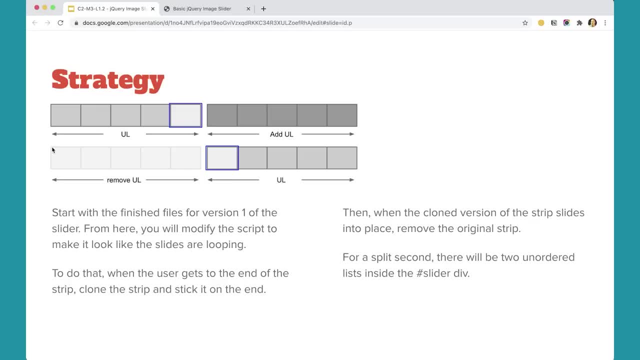 We've got five of them here, So it's going to go from 2,000 pixels to negative 2,000 to negative 1,600.. And that will push this first picture into our slider. And then this one is going to go from 0 pixels to 400 pixels. 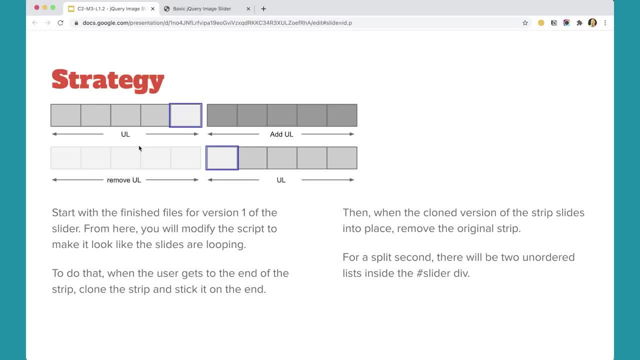 to move that there. So hopefully the diagram helps with sort of thinking about how this works and doing this kind of thing, And maybe you drew your own diagram in trying to solve this problem. Okay, let's go back to our slide with our answer. 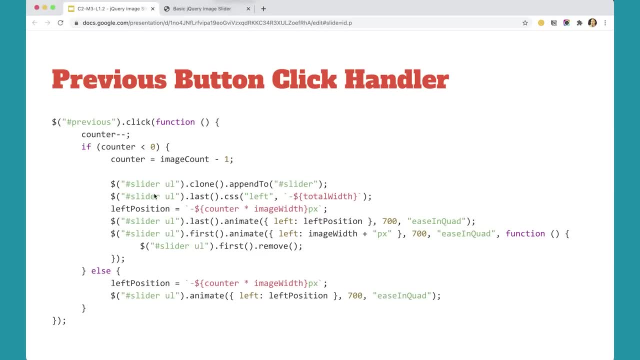 Here we are with our script here. So again, hopefully that image in your mind helps you. I know it helps me because I'm a visual person. But we're going to clone our unordered list, like we did in the previous one, But I'm going to set the last. 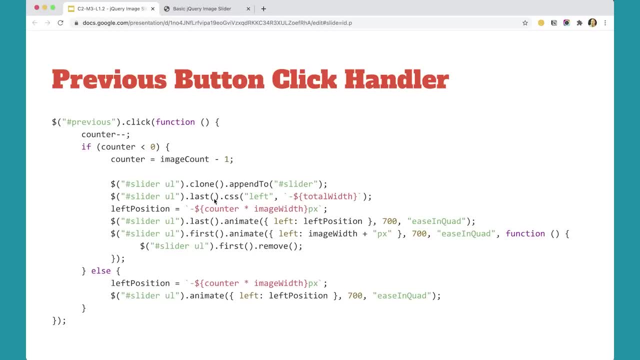 that last one that I've added into my DOM, the one that I've appended to the slider. I'm going to set the left to minus total width again, So that sets its left corner at that minus 2,000 pixel mark, right. 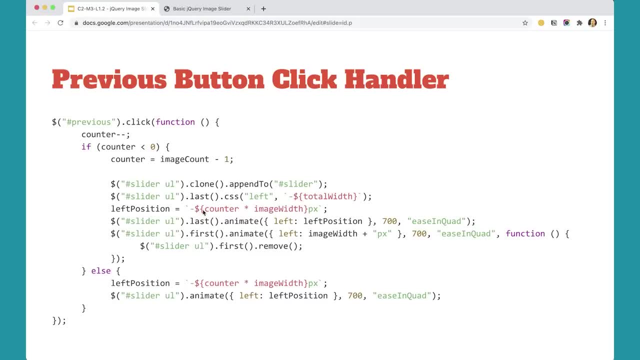 And we're going to set left position to minus counter times image width. So remember the counter got set to 4 here because it's image count minus 1.. Image count is 5.. We've got 5 images Subtract 1,, you get 4.. 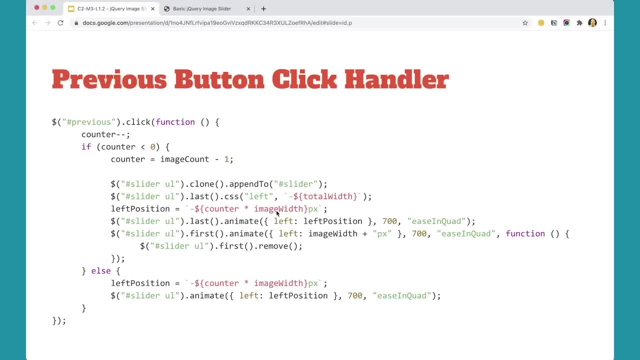 So counter is 4.. 4 times 400 gives us 1,600, right: 1,600 pixels Minus 1,600 pixels. And remember we're moving our strip from minus 2,000 pixels to minus 1,600 pixels. 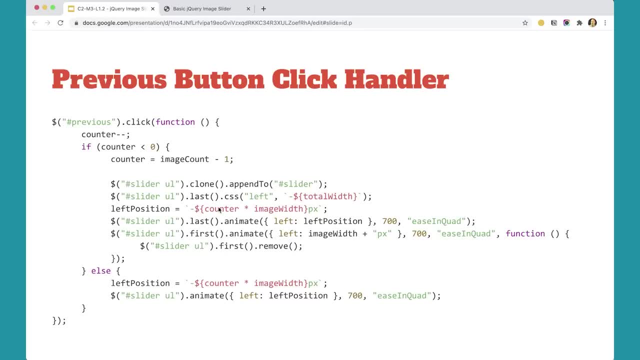 to move that left edge that's way over off the side there, into the correct position. So that's what that left position is going to be set for. So then we can take that last one and move it into the correct place. That moves that strip onto the screen. 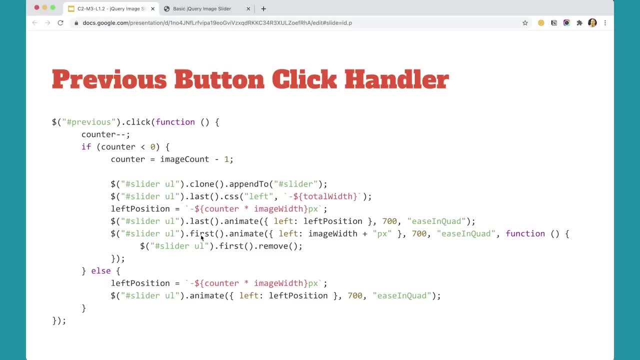 And then we take the first one and move it so it's off the screen, And then we can, with our callback function, remove that first one. So let's go ahead and do this on our script over here. So down here in the previous counter. 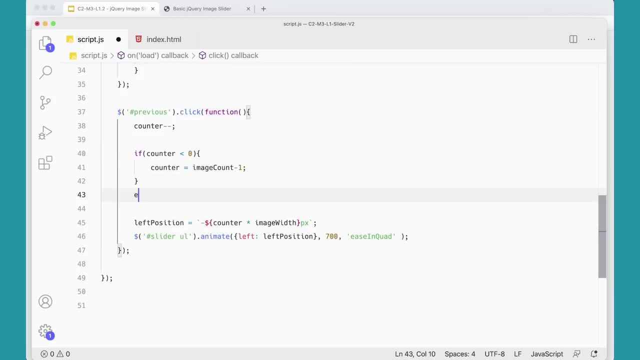 we're going to do the same thing we did before and add the else And move this stuff in here. So that's all going to happen to the else. We're going to decrement the counter and then we're going to set the counter. 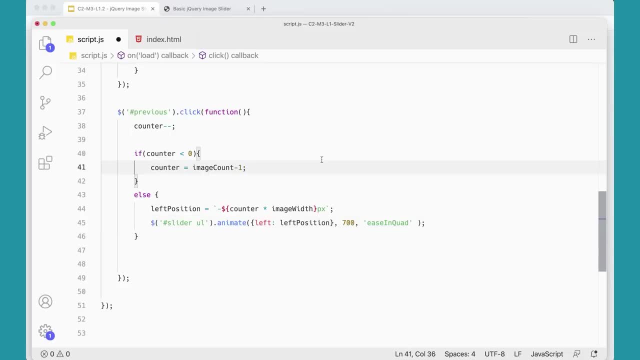 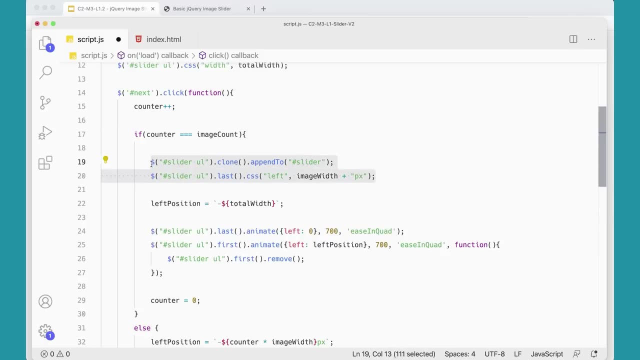 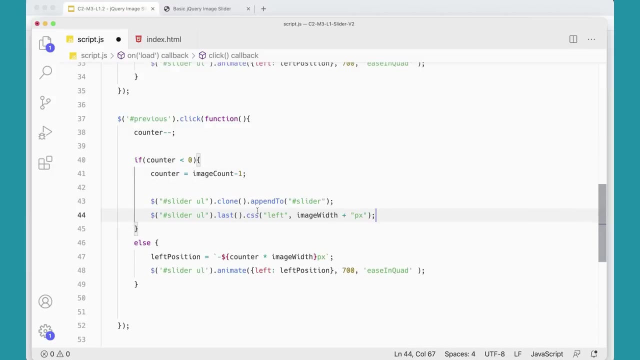 to image count minus 1.. So that all stays the same. Then we're going to do the thing that we did with the cloning up here, So I can actually copy this And paste it in here. But the position's going to be a little bit different here. 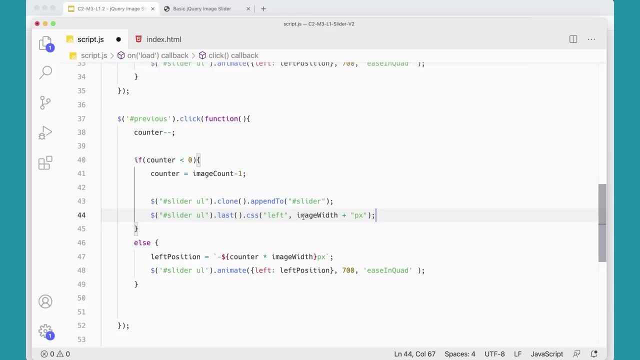 This position- the last one- is not going to be set to image width. Instead, it's going to be set to get my tick marks minus. oops, I'm going to put that in the tick marks minus dollar sign: curly braces. 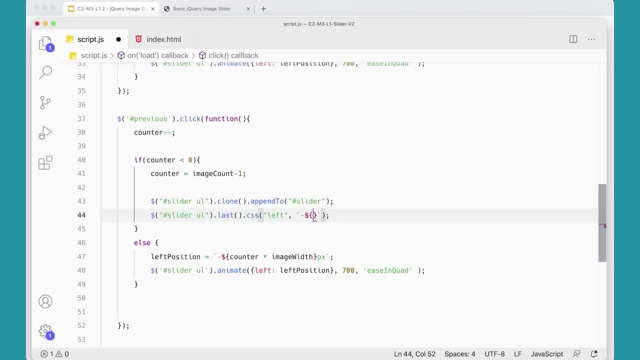 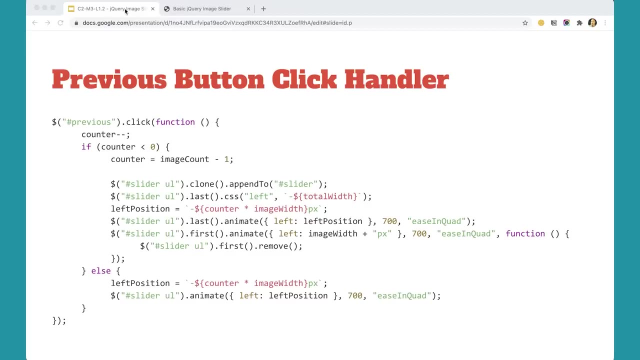 Curly braces- total width. I'm going to set it to minus total width. Right Left minus total width. Then I'm going to set the left position to counter times: image width plus the px. A negative for the negative number there, So let's put that in next. 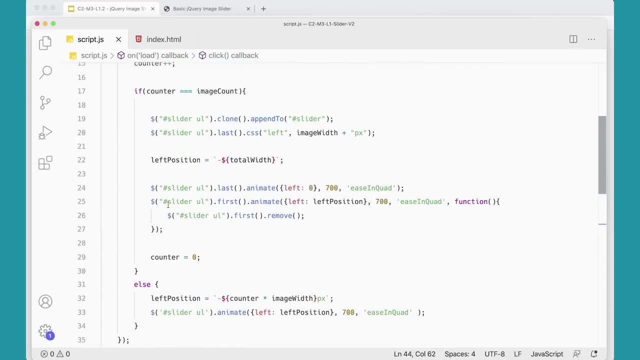 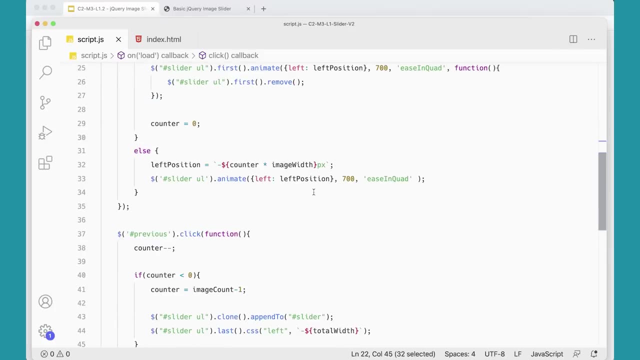 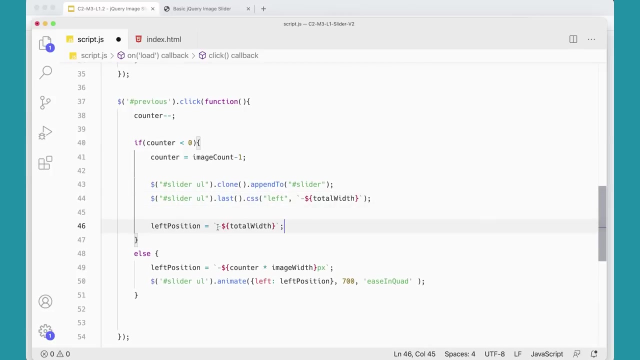 So that's really this line from up here. I'm going to put that in down here. But instead of just minus total width, it's going to be minus, it's going to be counter. what did I put? I've forgotten. 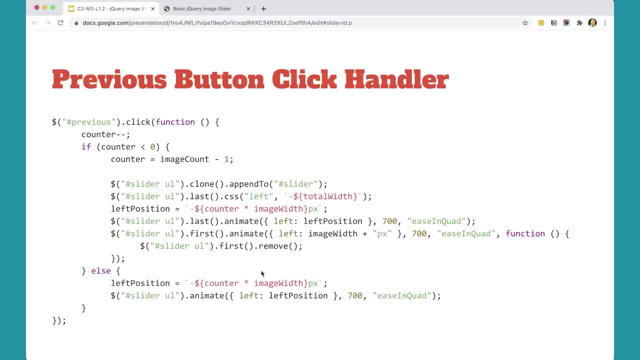 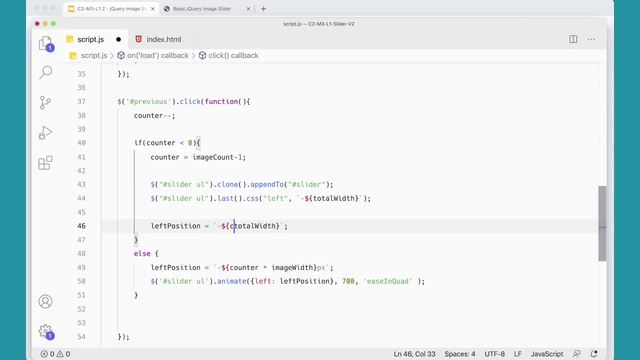 It's minus. then the counter times: image width. That's what it is. Counter times, not total width, but image width. There we go, Plus px. I'm going to need a px on the end of that, I believe. Yep, there we go. 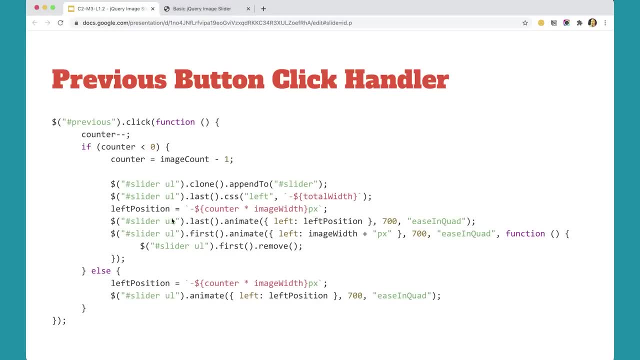 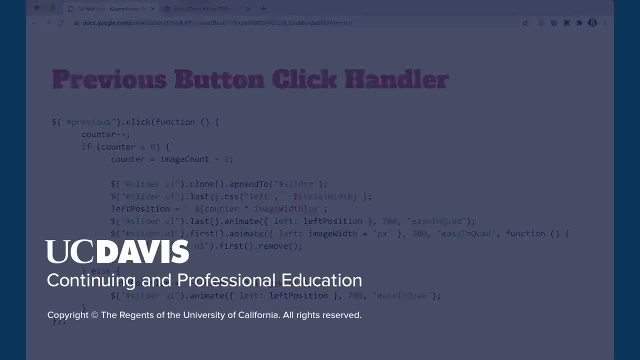 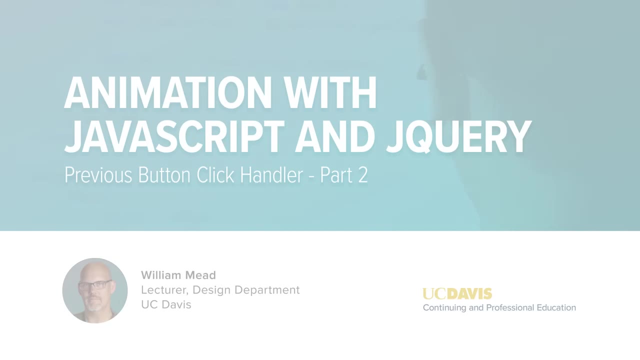 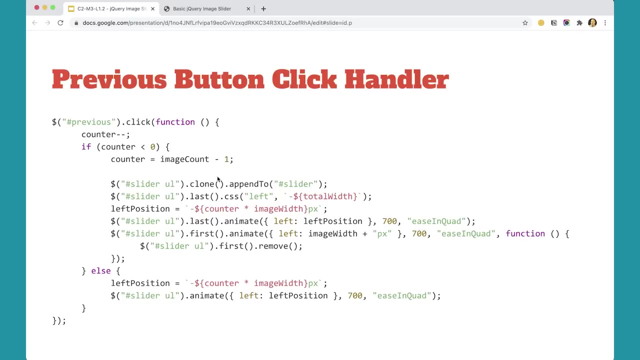 Okay, great. So then we just need to get get these two pieces in here, And we'll do this in the next video. In the last video, we worked out the logic of how the previous click handler is going to work, And where we left off was actually moving. 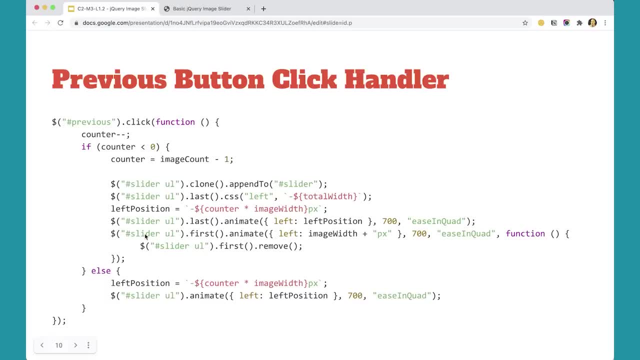 animating these strips into place. So that's what we need to do here. So we're going to take the, the unordered list that we cloned in there and animate it into its position And again, what we're doing is we're moving it from. 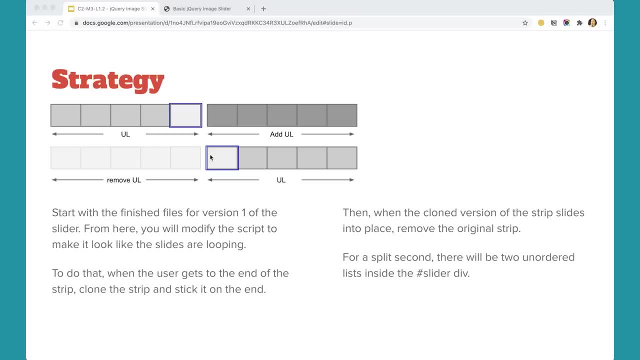 this position here. We're moving it from this position into here And the corner we're tracking is this corner over here. So this corner, when we added it to our DOM, is set to minus 2,000 pixels, because these are 400 pixels wide. 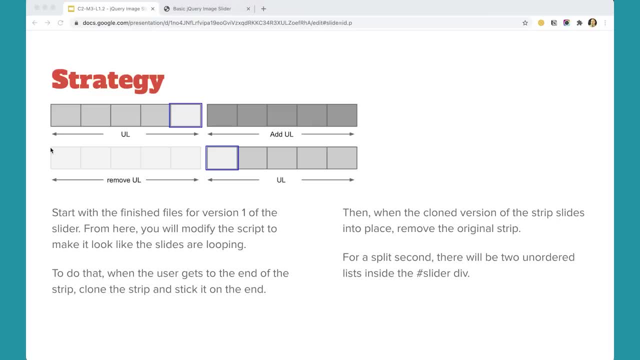 and there's five of them, So it's at minus 2,000 pixels. So we're going to move it from minus 2,000 pixels to minus 1,600 pixels, which will move it over 400 pixels, which will push the right side of this into our slider. 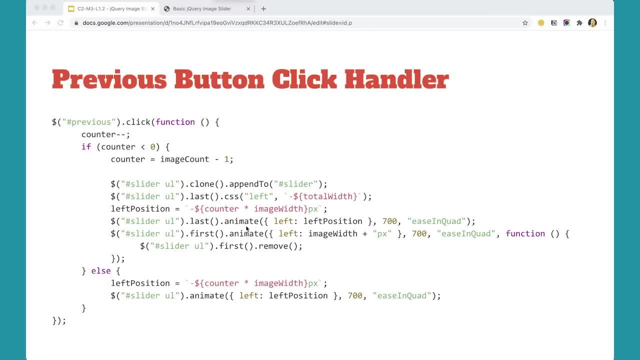 And you can see that's what's happening. here. We have our last element. we're animating to left position, And left position is now minus 1,600 pixels, over 700 using quad, So let's go ahead and add this line. 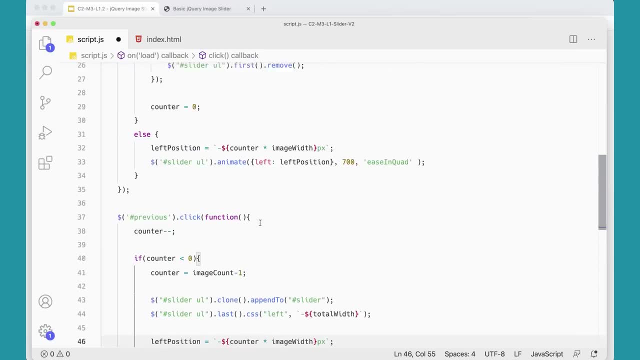 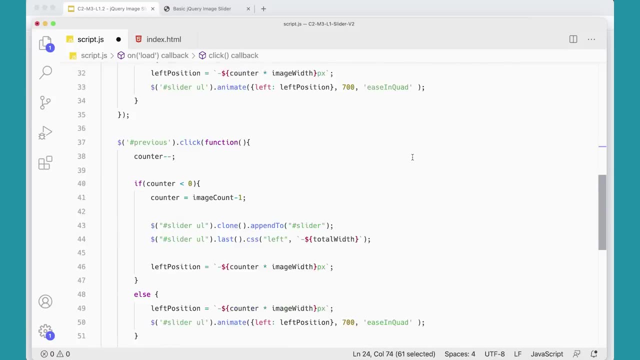 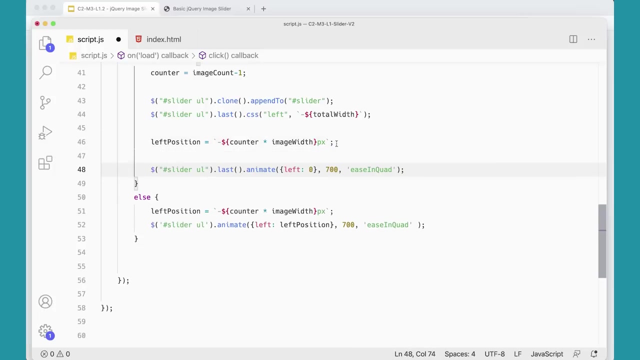 into our script over here And really you could actually come up here and copy this one And stick it in here. But instead of left 0, we're moving to left position, which is that minus 1,600 pixels The counter, which is 4,. 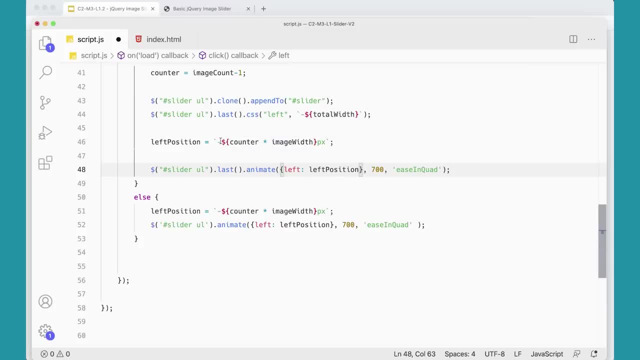 times image width, which is 400, that's 1,600, with the minus sign in front of it And with the PX. that's going to move that into the correct place. So that gets that one into the correct place. The other one. 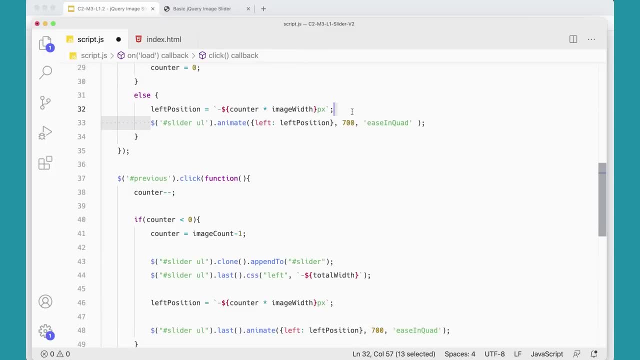 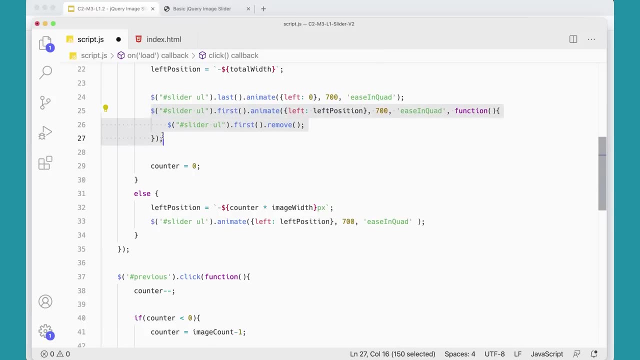 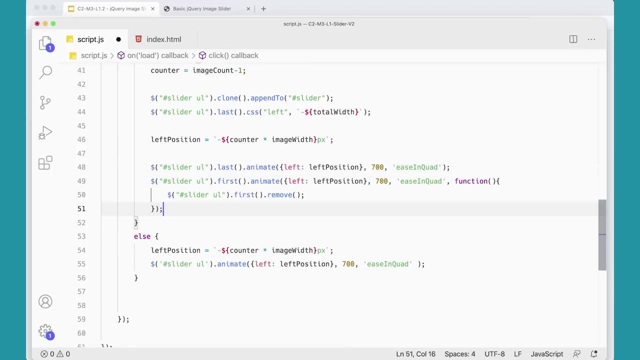 the first one, this one here, not that one, sorry. this one here first. We can actually copy this whole thing because we are going to remove it, So we can come down here and we can add that in here, But instead of moving it to left position. 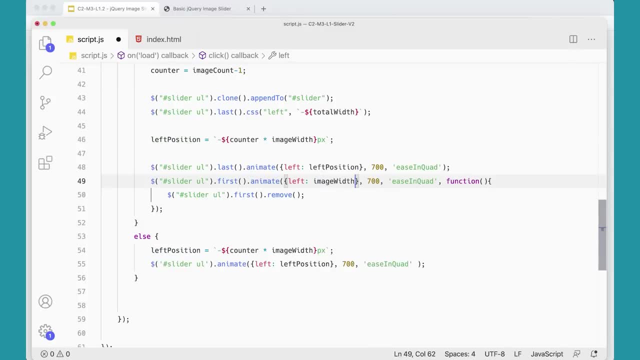 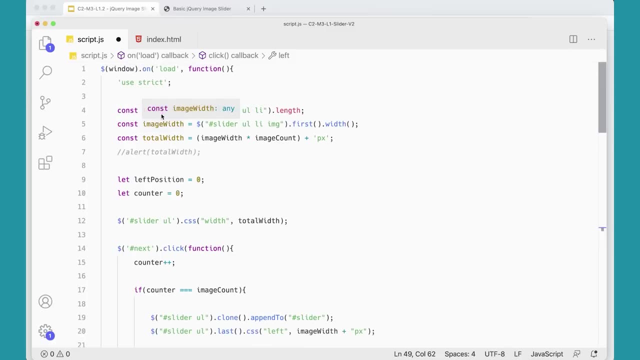 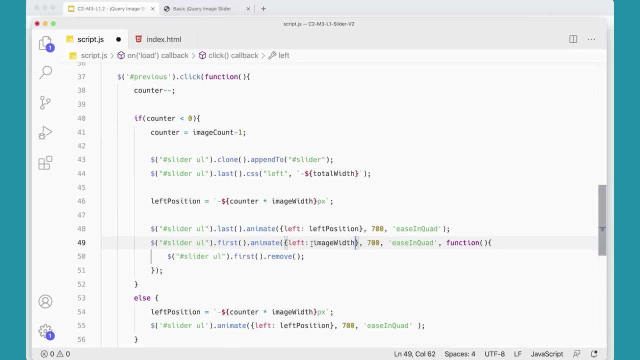 it's going to be moved to image width. Image width Which, up here the top of our script, image width is the width of that image, So we're going to need a PX on there. Image width. Let's do our tick marks. 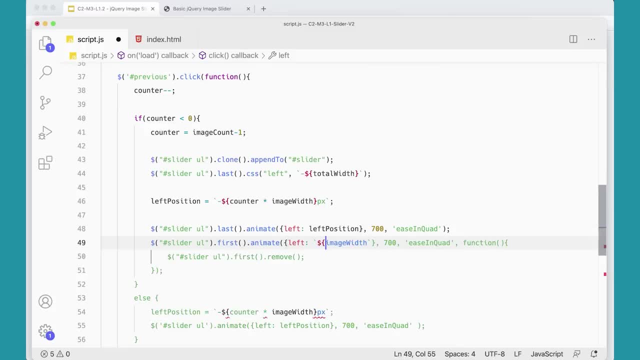 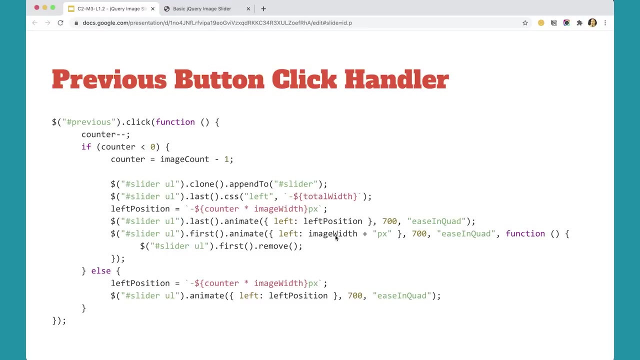 And then I can do dollar sign, curly, brace Image, width, PX Like. so I believe. Is that what I had over here? I have plus PX. I'm adding it on there. You can do it either way With the template, literally. 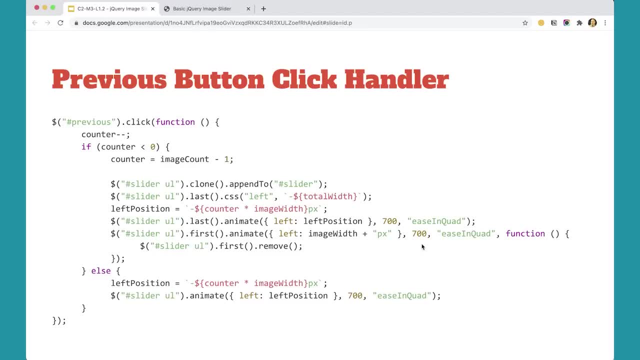 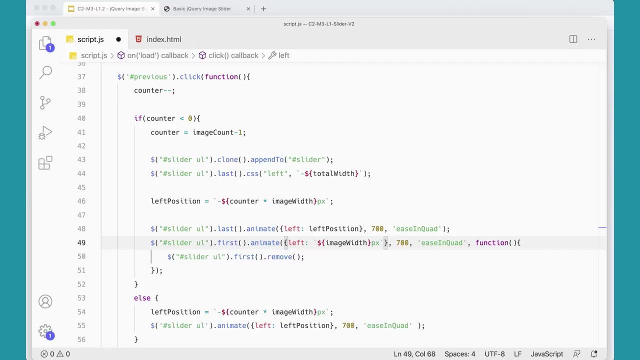 you could add the PX in there like that, And then we're doing it over here Over 700 milliseconds, Ease in quad. And then we've got our callback function again to actually remove that first one from the list. Let's see if it works. 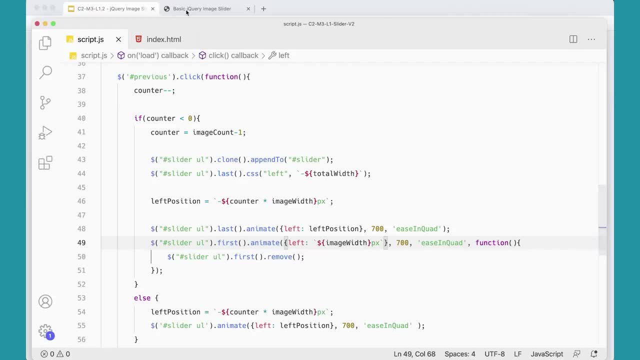 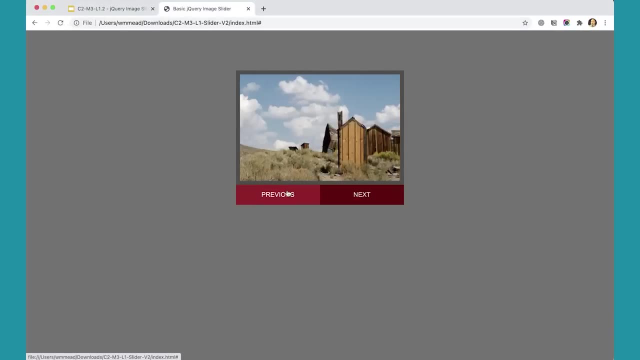 I'm going to save this. Come back here, Refresh it. We know the next one works, But does the previous one work? Here's our first slide And boom, it works. Here's our fifth, fourth, third, second. 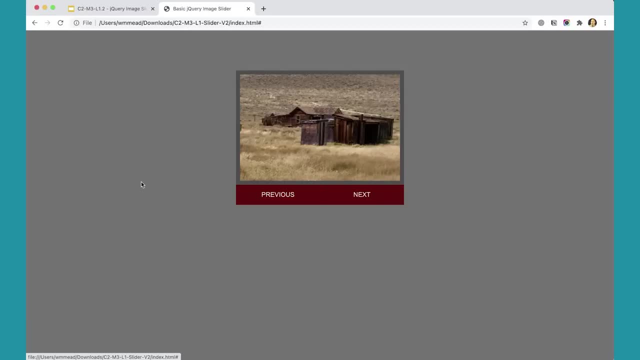 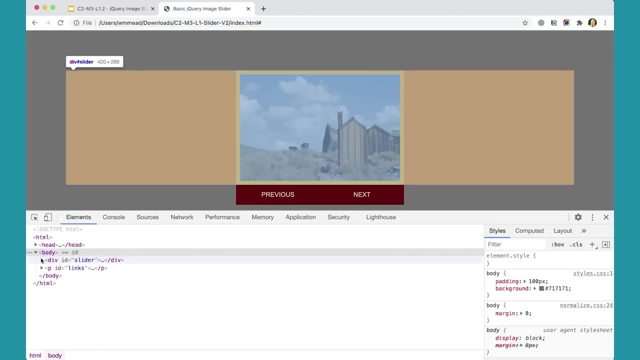 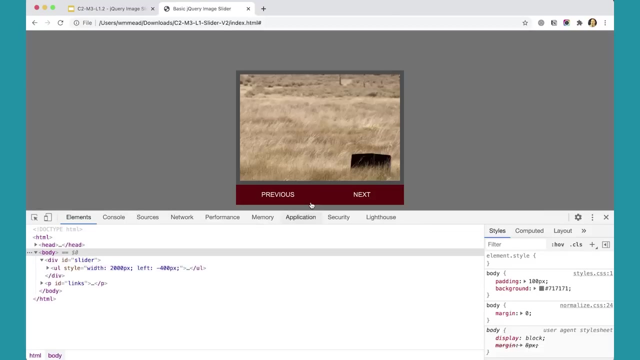 first and once again, boom. We can go around that way. If you choose the inspector, you can see it actually working. I've got my slider here. I've got my unordered list inside of there. Click next. You can see that's going to minus 400.. 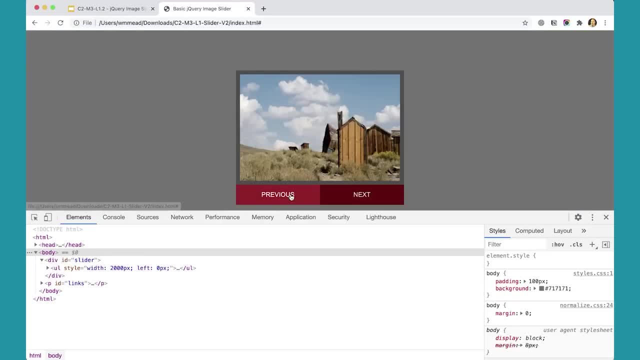 Click previous, It's going to zero. When I click previous again, you'll see it: add the unordered list, move it into place and then remove the other unordered list. So that's actually working exactly the way it's supposed to. So that's great. 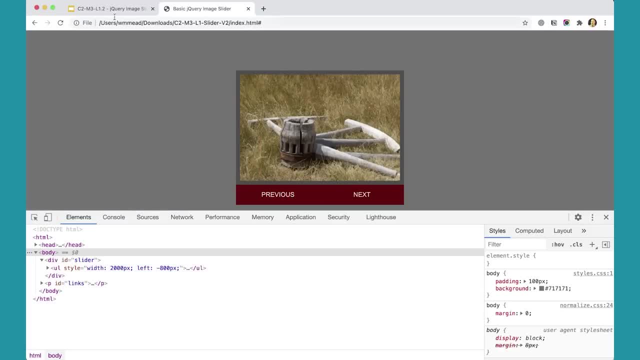 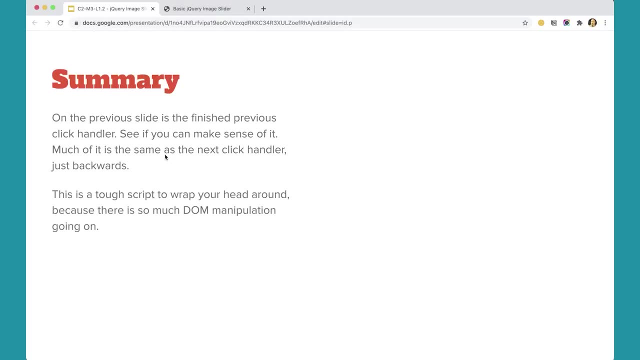 Very cool. So that's all working the way it's supposed to. There you go. Now you have a slider that will work in a looping kind of way, rather than just a strip that moves back and forth. It seems a little bit more complicated. 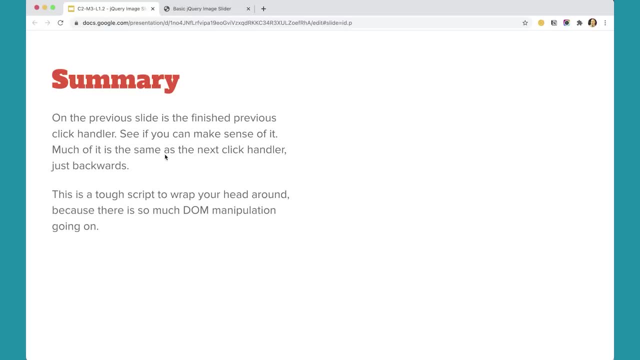 and it is a little bit more complicated, But these types of projects and these types of lessons are really helpful for thinking about different ways and different kinds of things that you can use on your websites and build that will make use of jQuery, make use of the built-in effects library. 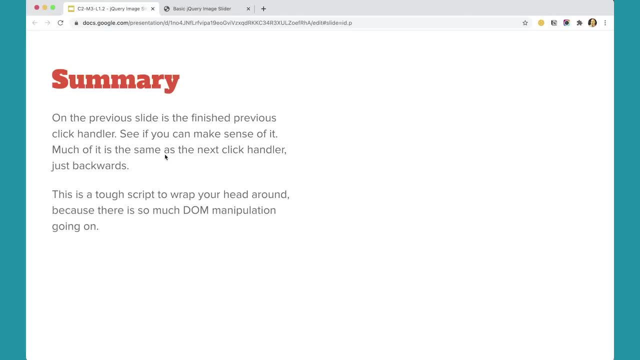 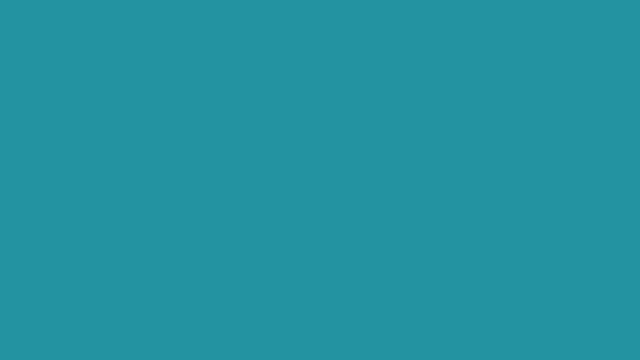 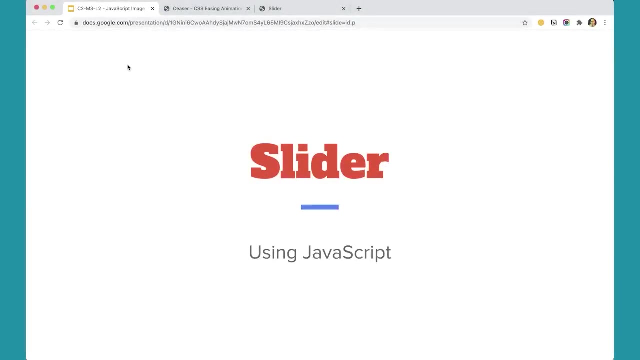 and teach you how to handle and think about these different types of situations that come up. Slider Using JavaScript. In the previous lesson we worked on making a slider using jQuery. We did a couple versions of it. Here we're going to do the same thing. 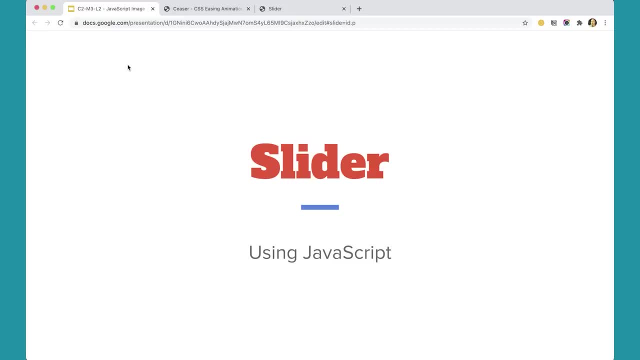 using plain JavaScript without jQuery, just so you can compare the syntax and see how different it is. There will be a few little minor differences in the script, but it's very similar to what we saw with jQuery, So that'll be pretty exciting. 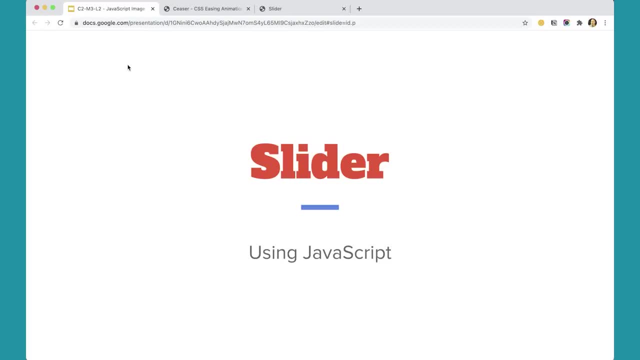 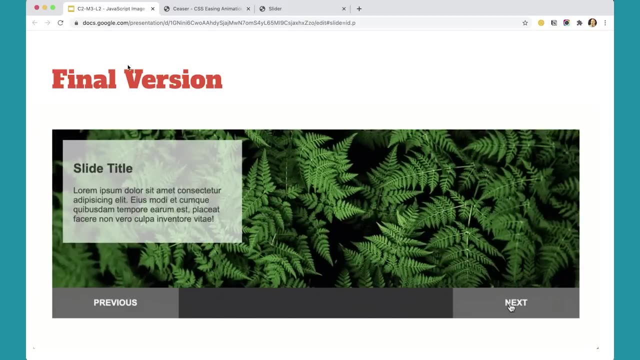 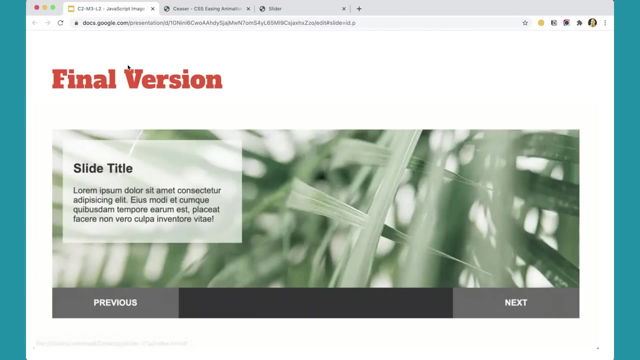 Here, the animation is going to take place in CSS, and we'll be using JavaScript to trigger the animation. In the end, you should get a slider that looks like this: It's a little bit different in that the slides are going to have some actual content on them. 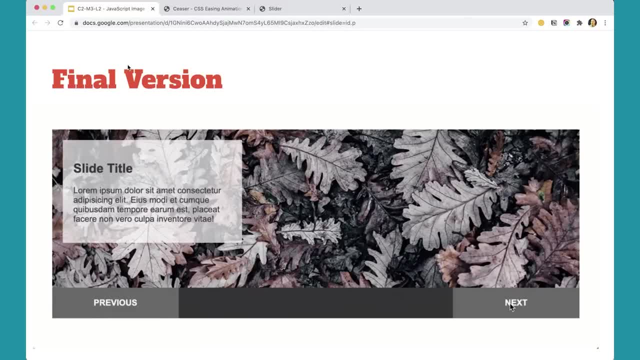 So they will have. The pictures will actually be in the background of the slide, and then they're going to have a little bit of a title and some text on them. So let's take a look at how that's set up. The basic strategy is the same. 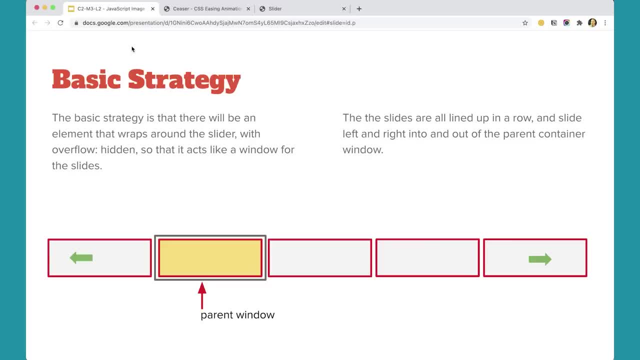 in that we're going to have a parent window that has overflow hidden set on it and that's going to act like a window for these slides. and the slides are all set up- In this case I have them floated- and they're all set up to float next to each other. 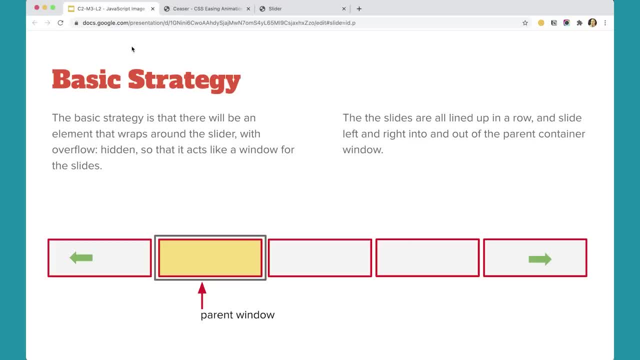 so that they end up in one long strip and as you click on the buttons, either left and right, the strip of slides moves in and out of the parent window, showing only one image at a time. There's our basic strategy, very similar to what we had with the jQuery version. 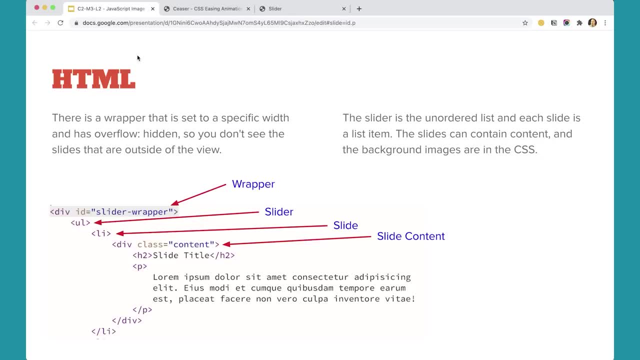 Now the HTML is a little bit different in this case because, instead of the list items just having a picture in it, like what we had for the jQuery slider, the list items have a div inside of it and the div is going to have an h2 and a paragraph inside of it. 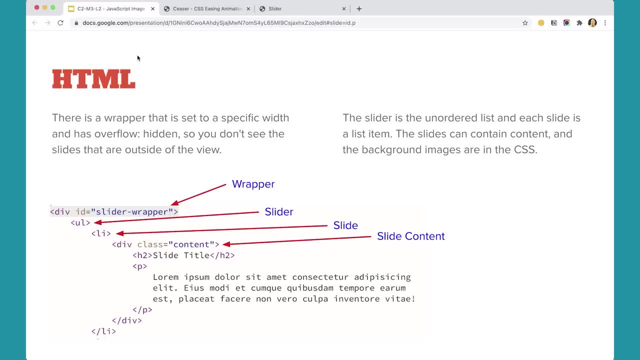 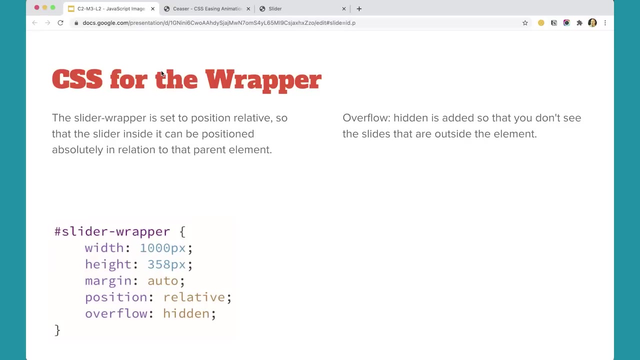 to create some content on that slide. The actual picture will be in the background of the list item, so that the list item is actually showing the picture as a background image. Now let's take a look at the CSS for this slide. Let's go to the wrapper. 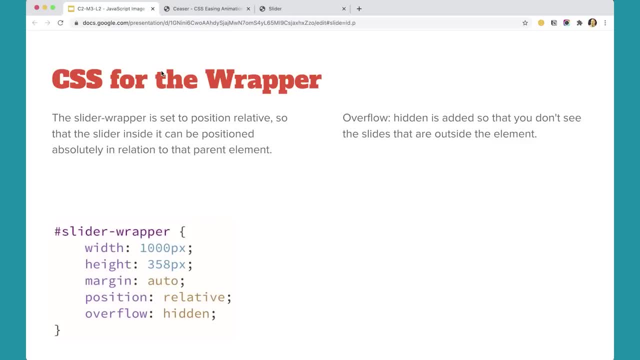 The wrapper has a width of 1000 pixels and it's set to a height of 358 pixels, which is really the size of my pictures, And I'm setting margin auto on it to sort of center it on the screen and then position relative. 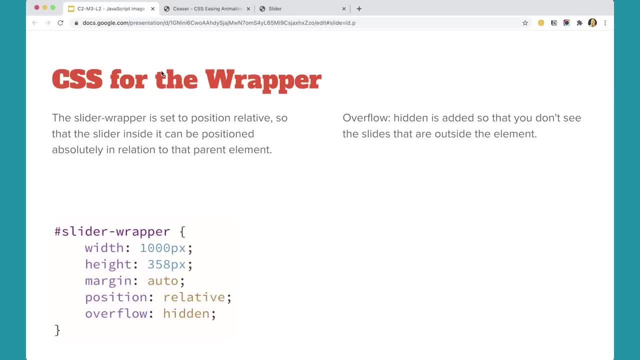 because we're going to absolutely position that string of pictures inside this window. This is the window that's going to show only one image And then overflow, hidden, so you don't see the other pictures. So we can come over to our code over here and see this markup in place. 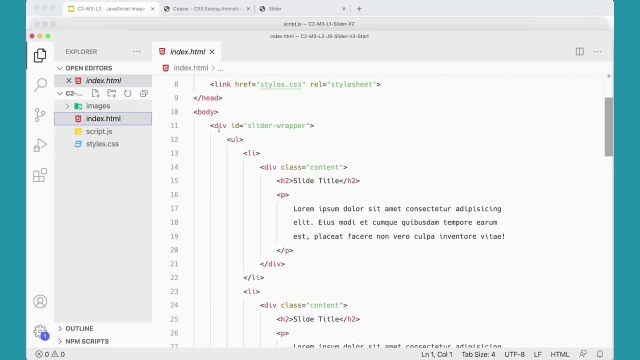 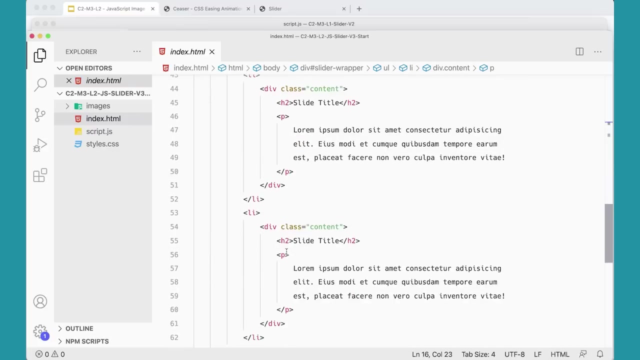 So you can see here I have my div with this slide wrapper, slider wrapper. I have an unordered list with a list item. The list item has the div with the content which includes an h2 and a picture, and I've got a bunch of these list items in here. 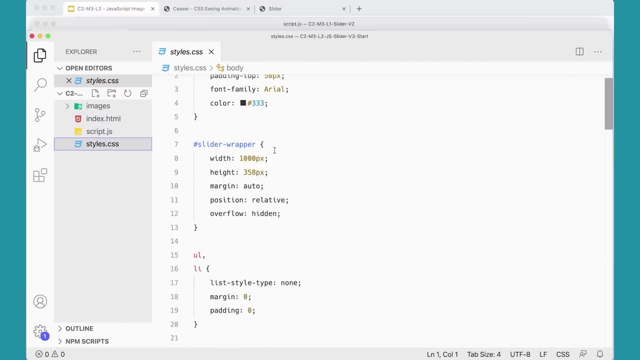 On the CSS, you can see that I have slide wrapper here set to a width of 1000 pixels and the height for the picture And then margin auto to center it, position relative and overflow hidden Down here as you look down through the CSS here. 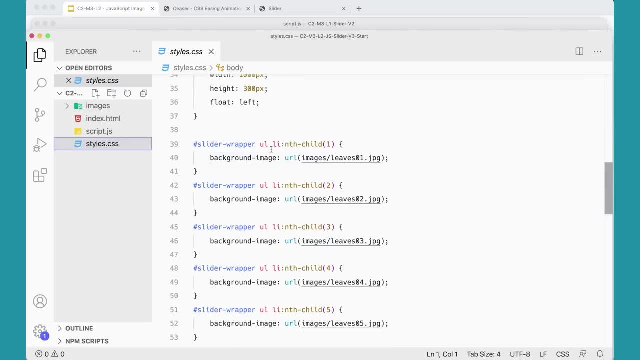 you'll see. this is where the background images are. It's on the list item. So the first list item gets this background image. Second one gets that one. The images are here in the folder, So I have all of my images here. 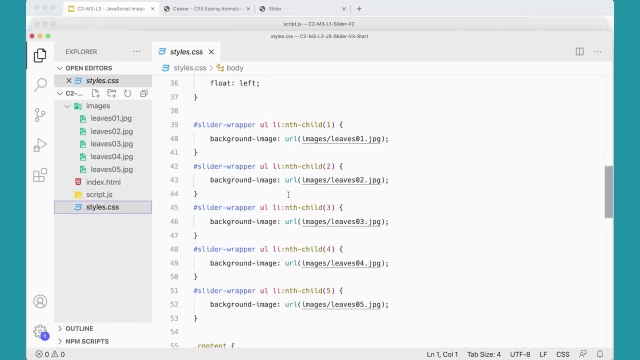 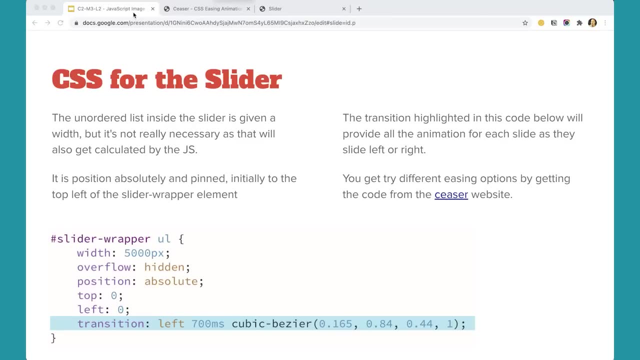 So everything will sort of line up and go into place that way. The actual animation is happening in CSS, So you'll look. you'll see this transition left: 700 milliseconds cubic Bezier with a bunch of numbers in here. 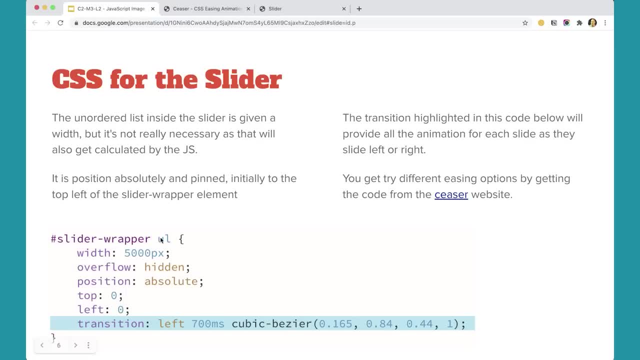 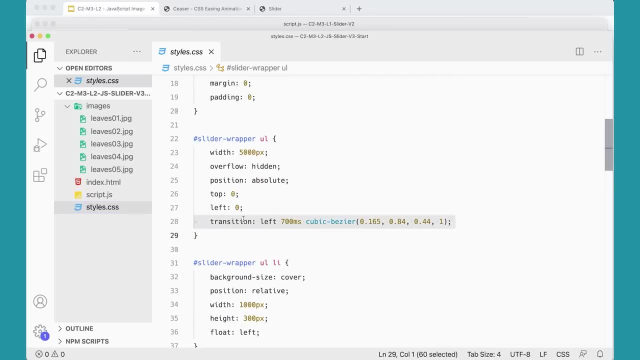 And I'll tell you about where those come from in a minute. But we can see this in our CSS over here, Right here. Using this transition, we're going to transition the left property over 700 milliseconds. That's the same as what we had in the jQuery version. 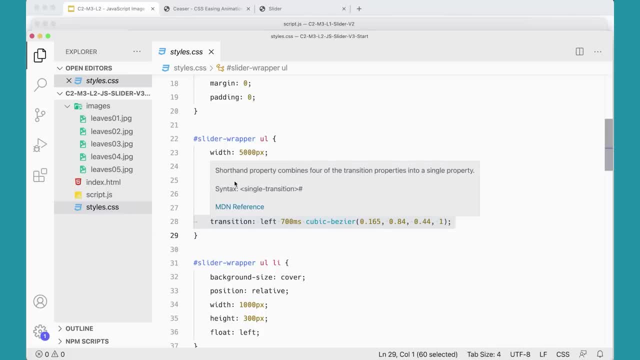 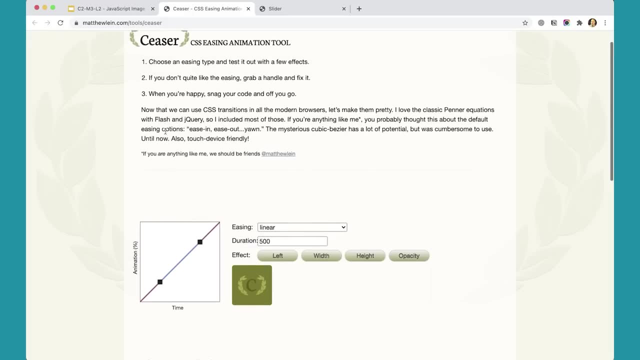 But this cubic Bezier? where's that coming from? What I used to create those is this little web tool called CSS Easer or Caesar. It's an animation tool, And you can see here- here's linear animation If I click left. 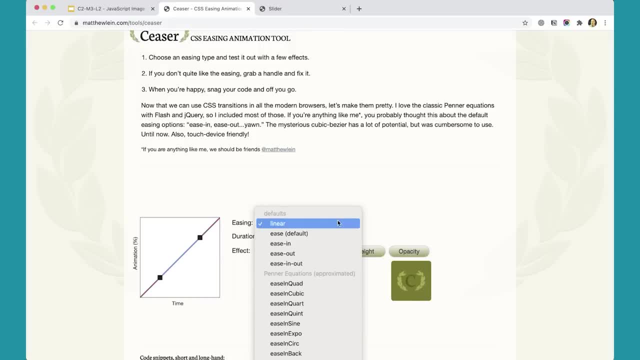 it just moves it at the same speed And you can pick one of these built in um options here to see what it looks like. We can change the amount of time. So that's starting slow and ending fast, Whereas if you were to do, ease out circ. 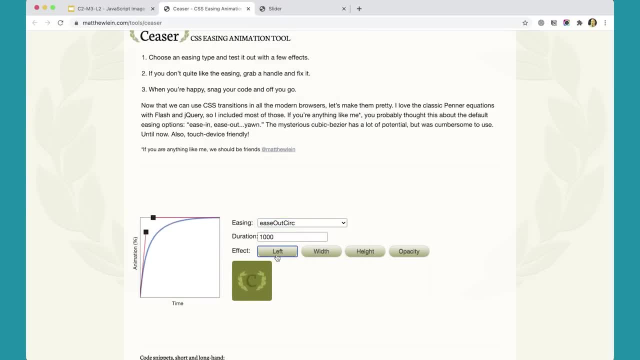 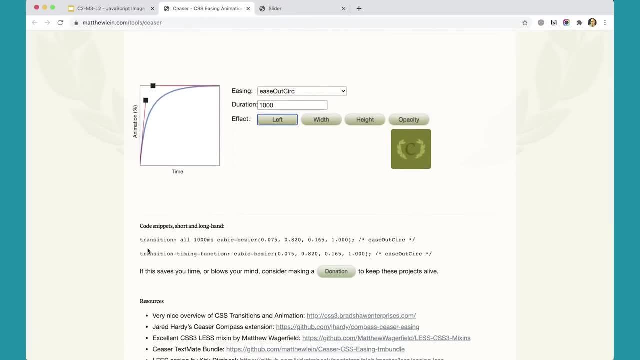 it would be the other way around: Start fast and end slow, And then down. here you can see the CSS that you actually need for this Transition all. But instead of transitioning all, I'm just transitioning left. But you can see that that's the code that we need in order to do this. 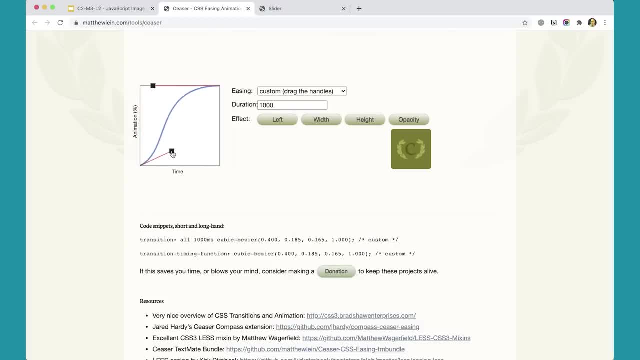 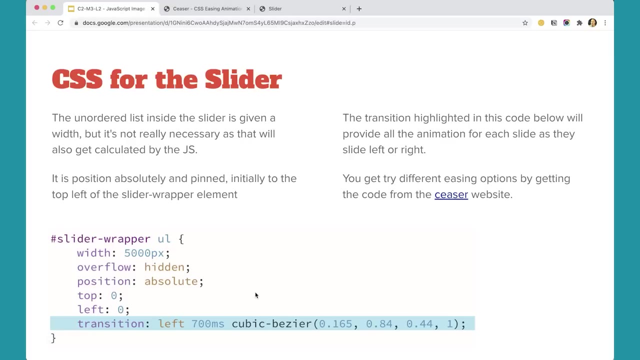 And you can even customize this. You can drag these handles and create your own customizing to do whatever you want it to do. Um, and it'll adjust these numbers accordingly. So that's where that comes from. So that's going to create the actual animation for the slides. 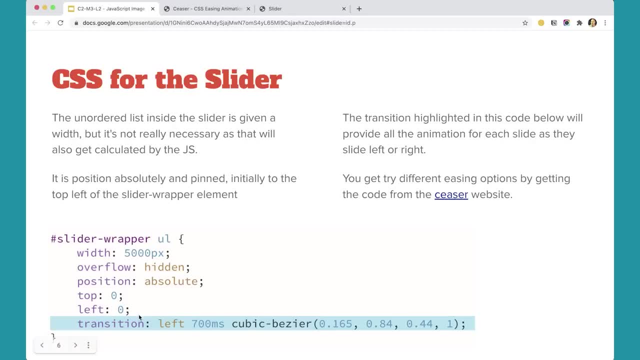 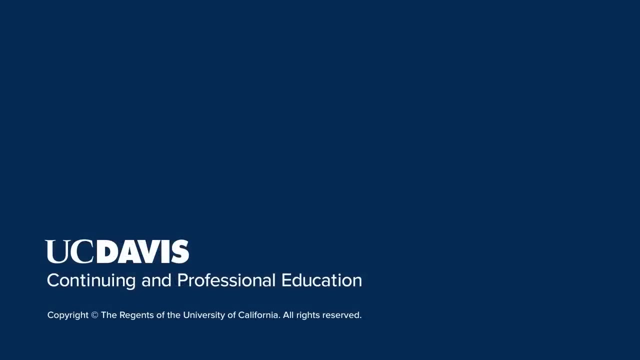 So, each time a slide moves, this transition is going to take effect. Each time we change the position of the slide- the left position- this animation is going to take effect. And, uh, that's where we'll see the actual animation for our slider. 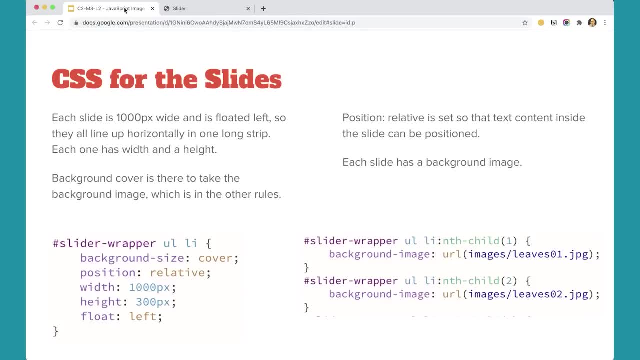 We have a little bit more CSS to talk about before we start working on our JavaScript, And the first thing is the actual slides themselves, So the list items that are inside the unordered list, that are inside the slide wrapper. which are these elements here in my index page? 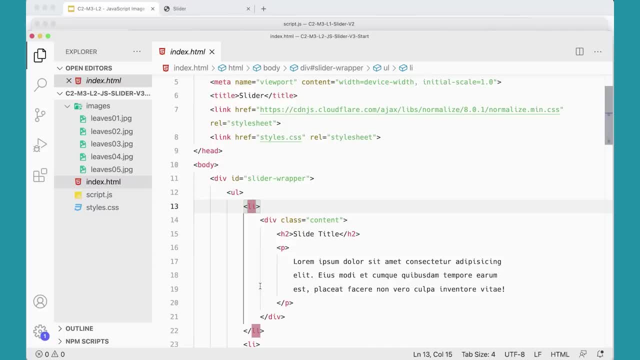 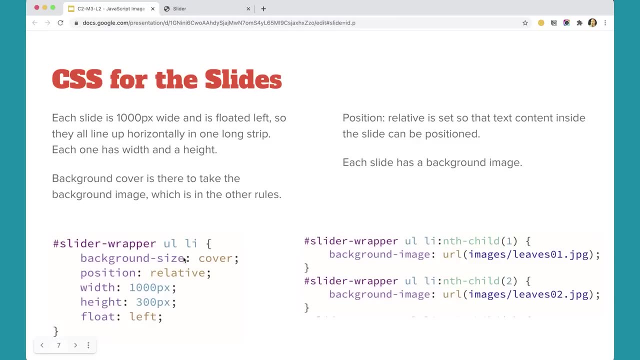 these list items here. These are my actual slides And I want to set some styling for those. First of all, I'm going to make sure the background image covers the entire list item, So even if they were to get a little bit cropped or something like that. 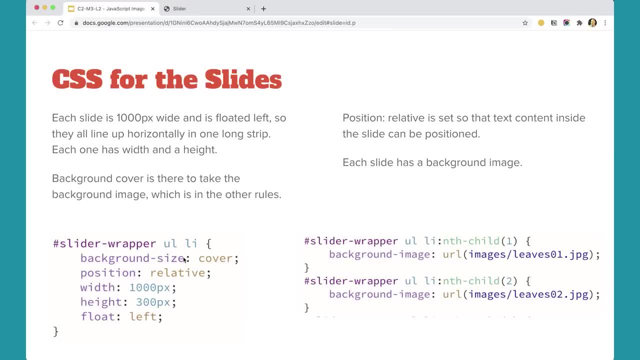 then that's fine. I want to make sure the image covers the whole thing, because it's a background image, as we see over here, And as we mentioned before, each slide, each list item gets its own background image, So those images go in the background and they 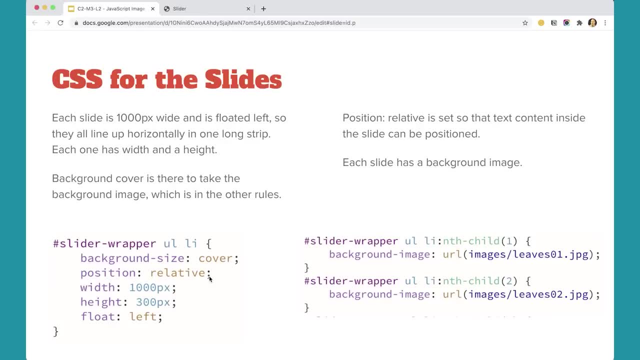 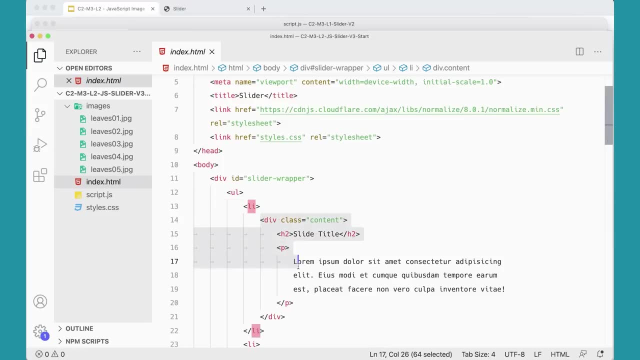 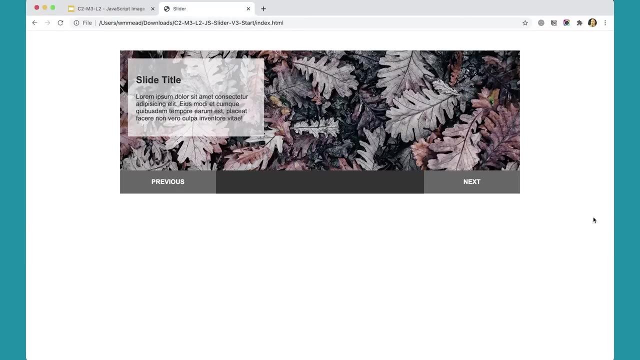 and they cover the background of that list item And then they're set to position relative, because the content that's inside these slides, this div with the H2 and the paragraph, is going to be absolutely positioned Basically, this div here it's going to be absolutely positioned here. 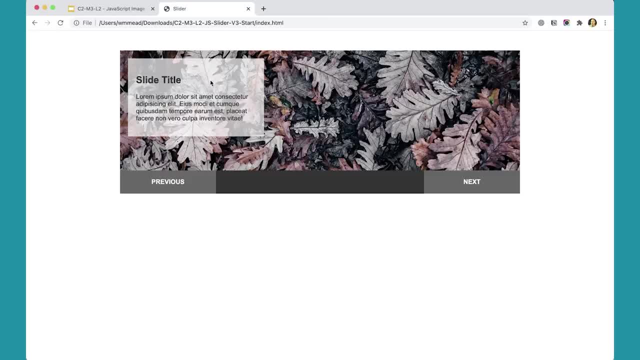 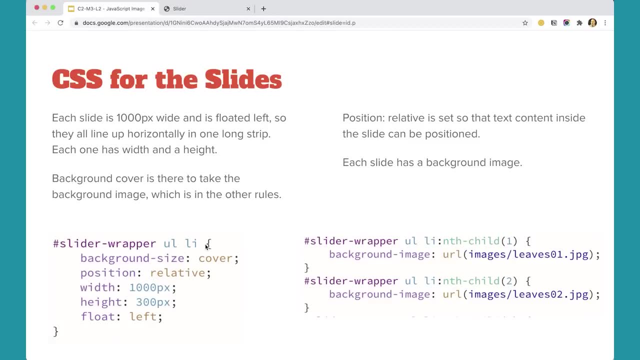 Um, so that it gets positioned on the slide Inside of the background there, um, on top of the background, So that gets so. um, these are set to position relative, because those divs are positioned absolutely, And then then we set the width of the slide and the height of the slide. 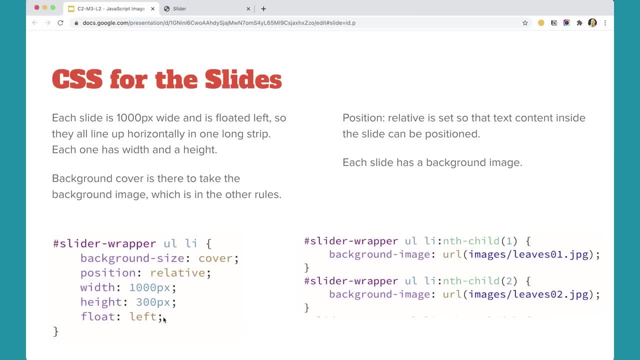 And I have them floated left, So they all go in a line next to each other, And, uh, that should make them all work pretty well there. Okay, So we've got all of that in place and and working, And now we're ready to. 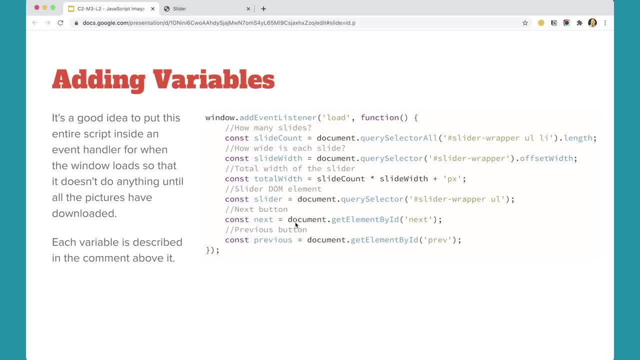 uh, start working on our actual JavaScript And for our JavaScript. in the jQuery version of this we use the on method to make sure that the window has loaded. We did an on load method, Um, and that was an event listener in jQuery to check. 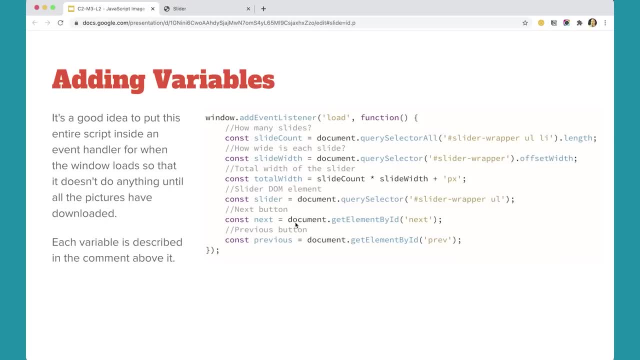 to make sure that all those images have loaded here. We're just going to add an event listener, We're going to add an event listener with the add event listener event And we're- uh, the added add event listener method and put it right on the window. 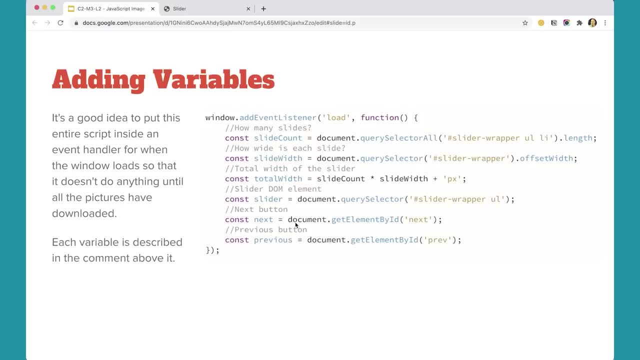 And we're going to check for the load event And that will also do the same thing where it's going to check to make sure that all the assets have loaded before it runs the callback function, which is the anonymous function you see on that first line of the script. 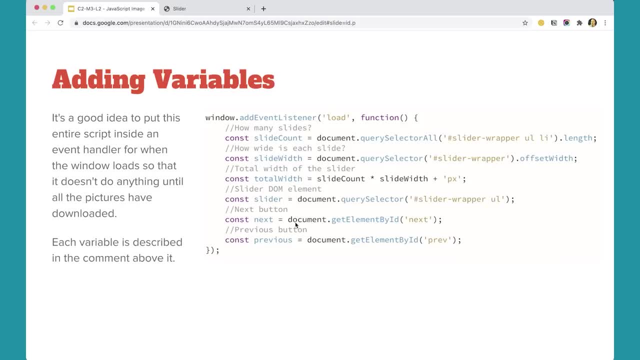 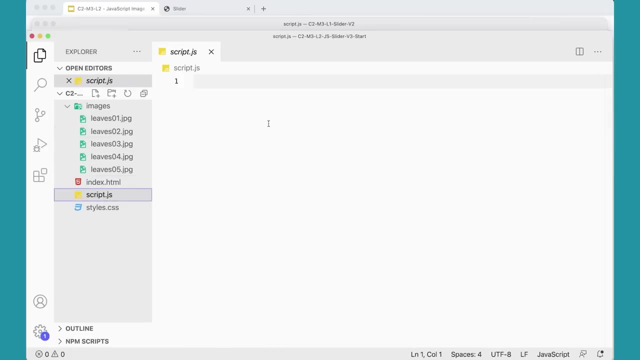 there And everything's going to happen inside of that anonymous function that runs after the page has loaded. So let's go ahead and add that event. listener to our script. First come over to my script file and I'm going to add a window. 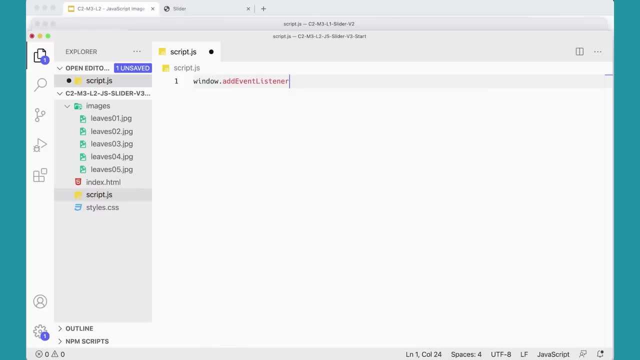 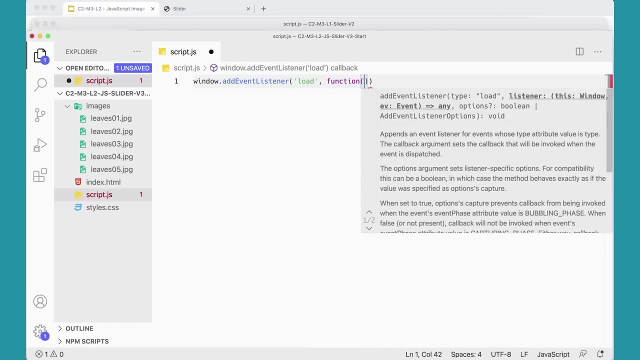 I can type it: window dot. add event listener And I'm looking for a load event comma. I'm going to run a function that runs when the page has loaded All of its content. So we're going to run that function And in here. 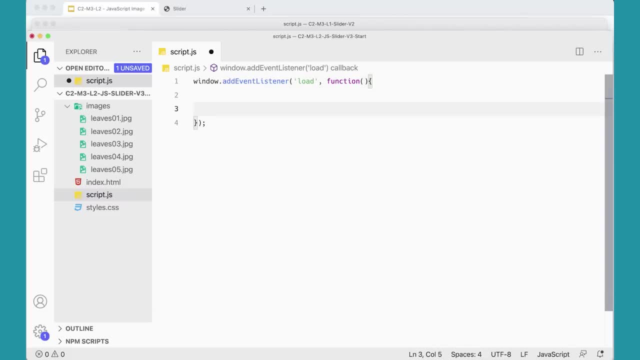 I'm going to add a number of variables, And a lot of these variables are going to look familiar because it's very similar to what we did with our jQuery version of the script. Also, this, uh, this function here will function as a 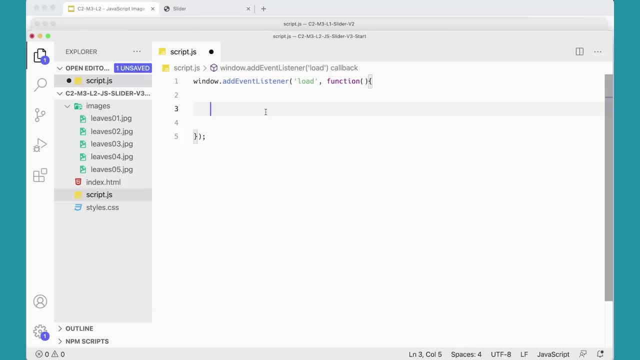 as a as a closure for this whole script. So I don't have to worry about adding an I, I, F and the invoked function expression, because this function will make sure all the variables, everything in here, are local to this function and nothing will be leaking into. 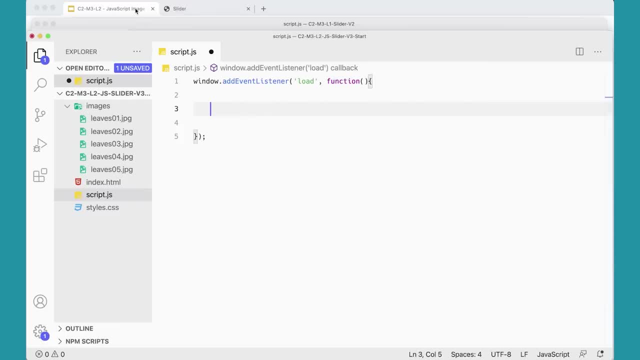 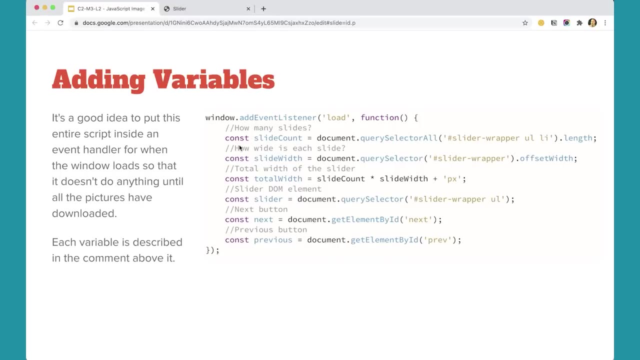 the global scope. So we don't need to worry about doing that for the script either, because we're putting it in this uh event listener for when the page loads. So what do I need to know? I need to know how many slides do I have? 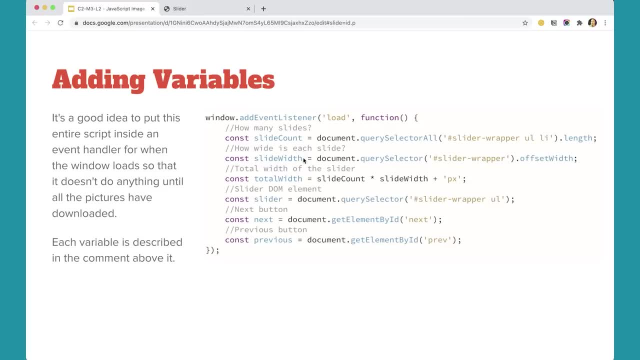 How wide is each slide? Uh w. what is the total width of the slider? Uh, and then I need to get some DOM elements that I'm going to work with on my page, The actual slider element itself. this just kind of makes some shortcuts. 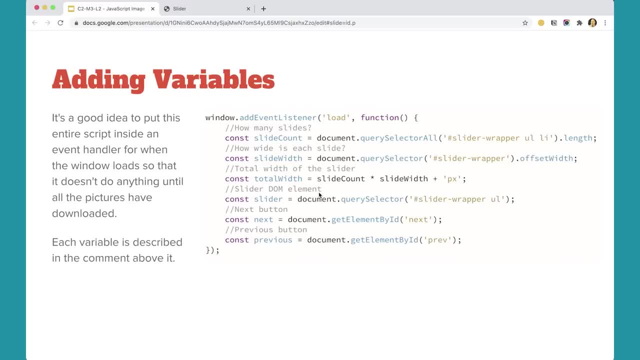 If I make a variable called slider, I don't have to type document dot query selector every single time I want to work with the slider. Same thing with the next button, previous button. So let's go ahead and add these in over here. 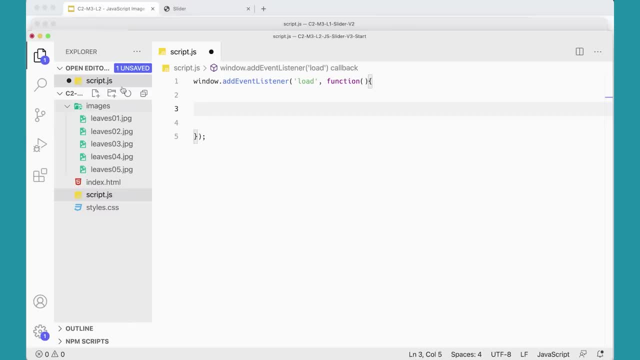 I'm going to go back to my script over here and, uh, I'm just going to paste this in. You're going to have to type it, but I'm going to paste it in. I'm going to make a variable called slide count. 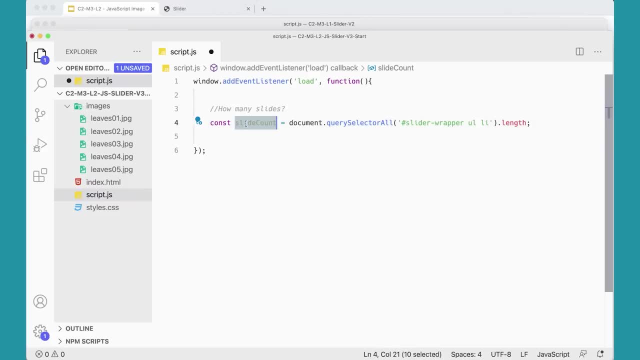 and I'm going to use query selector all to go and get the length of how many list items do I actually have? If I were to do an alert here, you'd find it. You'd get the number of list items that I have coming up. 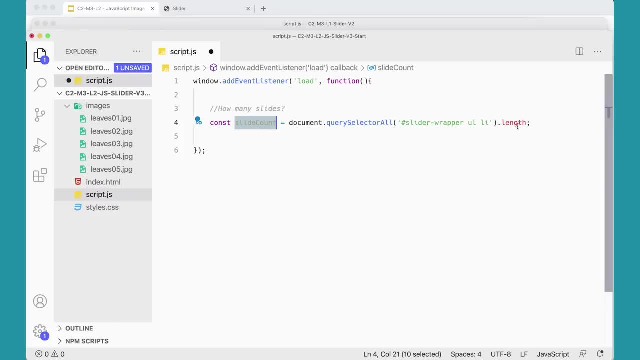 Let's do that real quick Alert. Okay, So I'm going to go ahead and paste this in. I'm going to paste it in. I'm going to paste it in. I'm going to paste it in Again. I'm having trouble typing today. 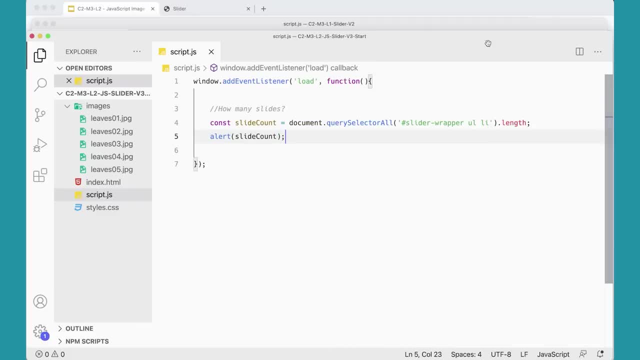 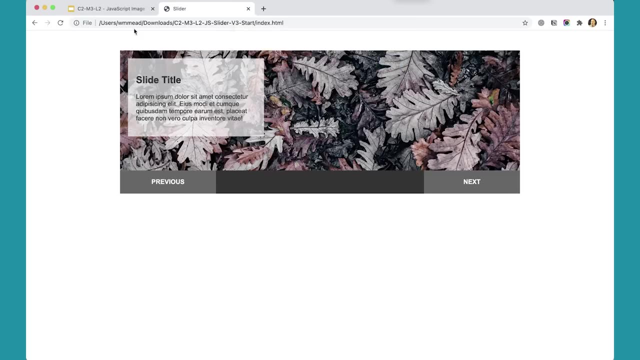 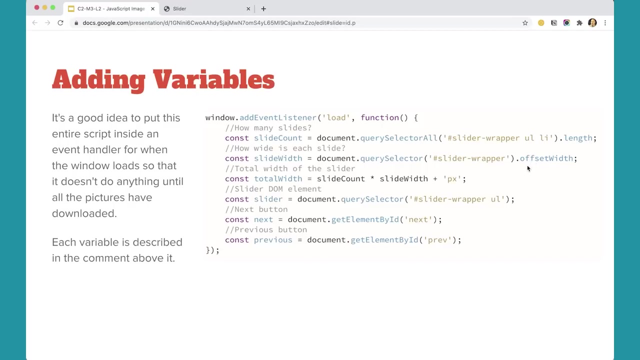 Uh, slide count. If I were to come back and refresh this, I should be getting a five. I've got five slides, So that's working. The next thing I need to know is how wide is each slide, And there's a property in JavaScript called offset width. 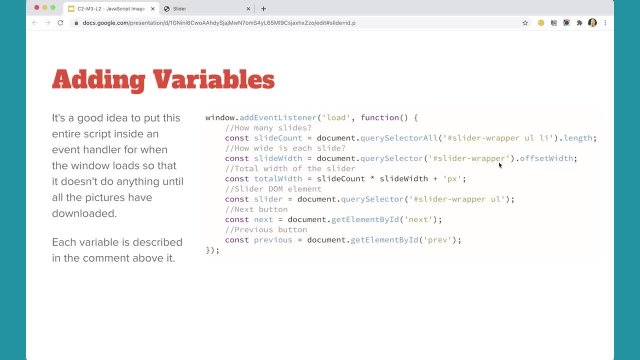 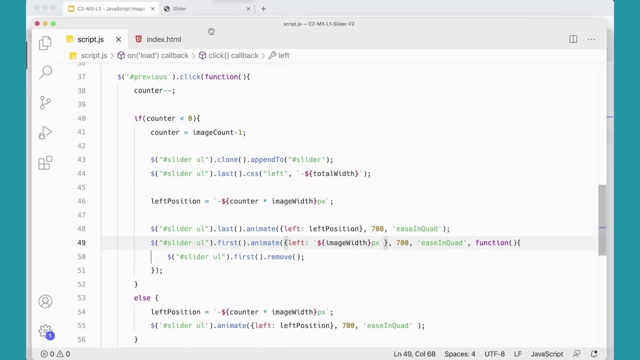 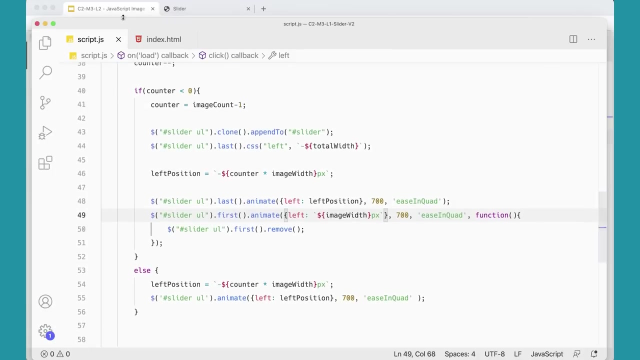 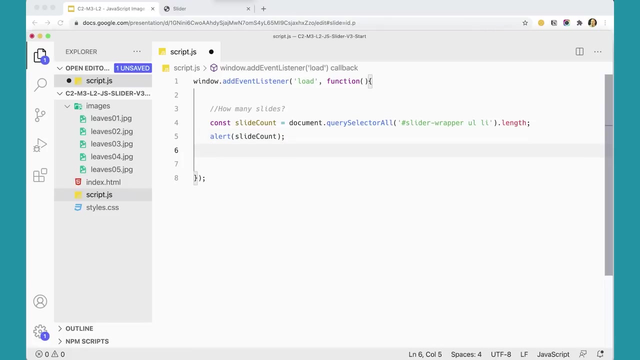 So I can go get this wrapper and say, well, how wide is my slider wrapper And that's how wide my width of my slides are going to be. So I can go and get that next over here. Oops, How wide is each slide. 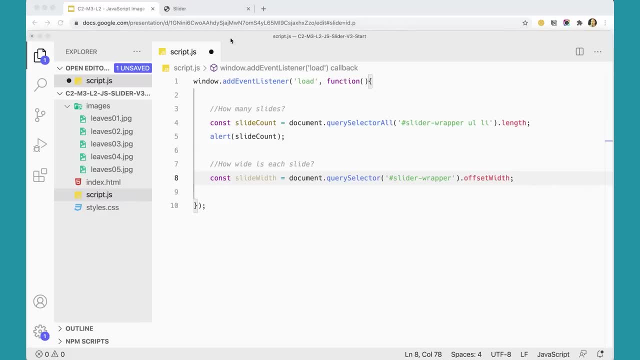 So I've got that. The next thing I'm going to need is the total slider width, which is going to be the slide count times the side slide width with the pixels. And then I need my Dom elements, which are these: the slider itself: 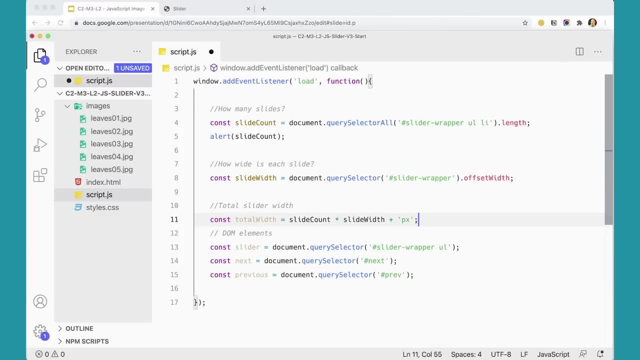 the next button and the previous button And you can get rid of some of the space in here if you don't want it, or even get rid of the comments if you don't want it. It does take up kind of a lot of room. 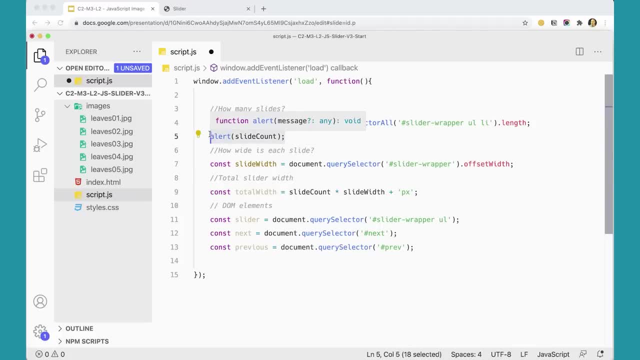 but, um, I don't need this alert anymore. I can get rid of that. There we go. So now we're set up, uh, with some basic variables here. We're going to need a few more variables to get before we really get started. 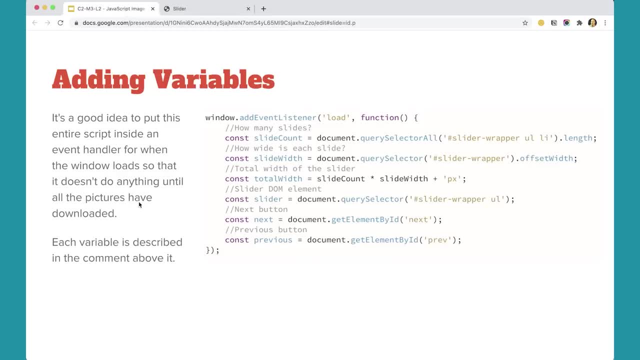 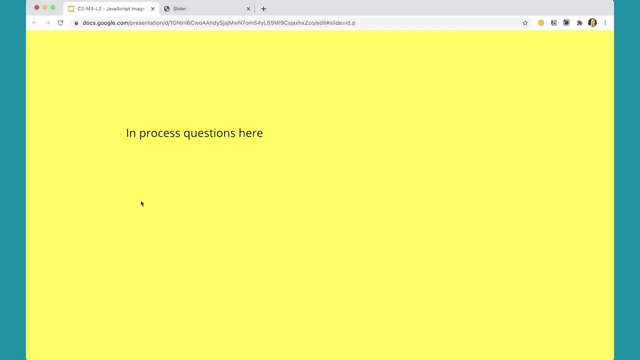 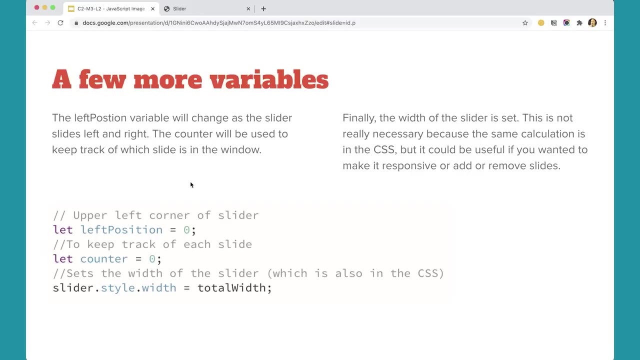 with our um, with our next click handler, Click handler. First, let's put in some questions here. Okay, Here are a few more variables that we need. We need to know, we need to use the let keyword because these variables are going to change. 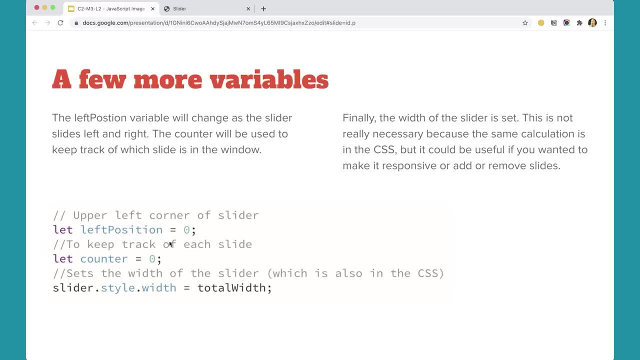 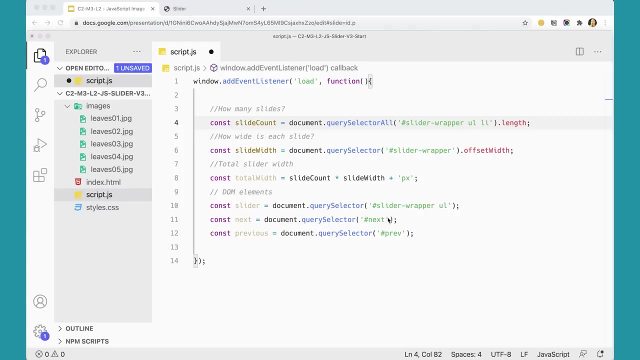 We need to get the left position and set it to zero. We need a counter, And then we want to set the slider style width to the total width. So let's go ahead and set those as well over here And again. I'm going to paste these in: 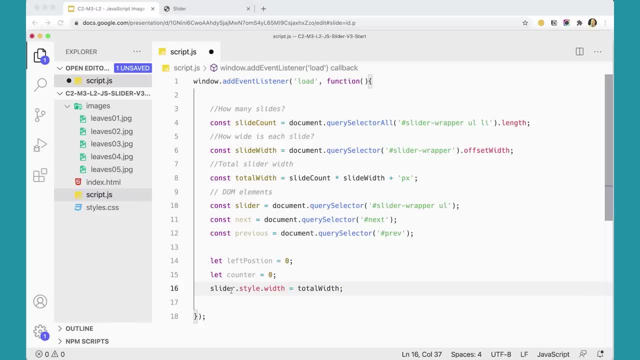 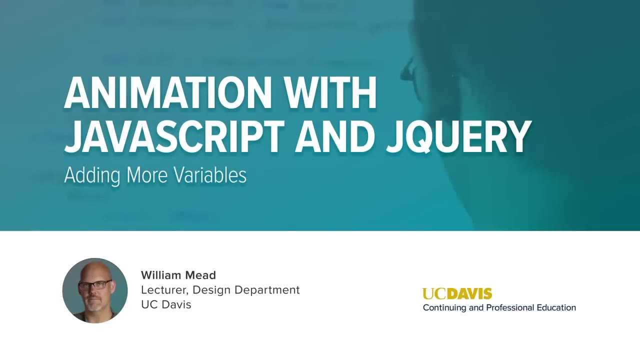 You're going to have to type them. So setting slider style that width to total width will actually set the width of that element And we'll talk about that and look at it a little bit more in the next video, In our last video. 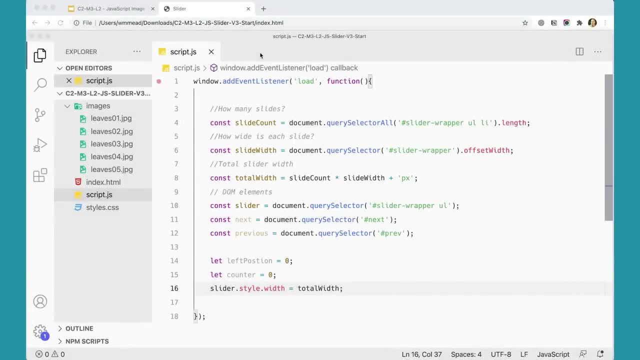 we got some basic variables in place for our slider and they're very similar to the variables that you saw for the jQuery version of the slider, But now we're using plain JavaScript, So the syntax is slightly different. It's a little bit longer. 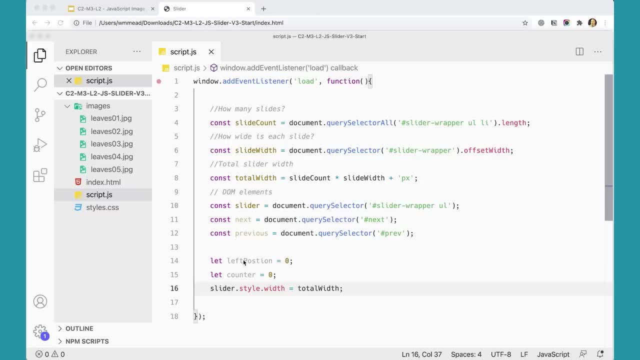 but it's not too bad. And here we've set the slider style width to total width And remember total width is the slide count times, The slide width of the PX, the end. And we're setting that locally in the style here. 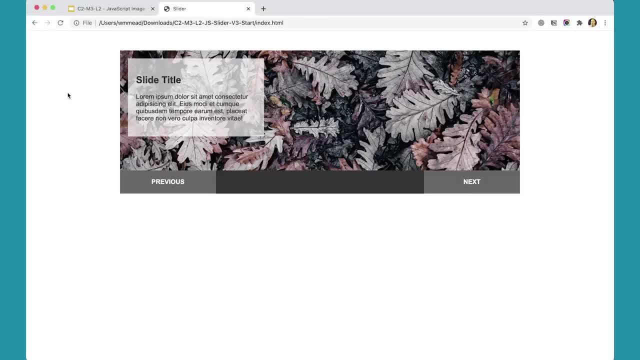 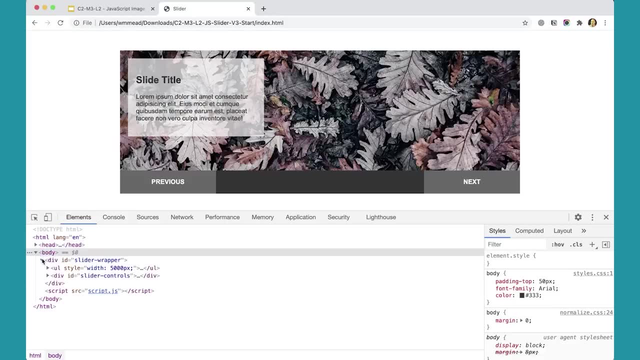 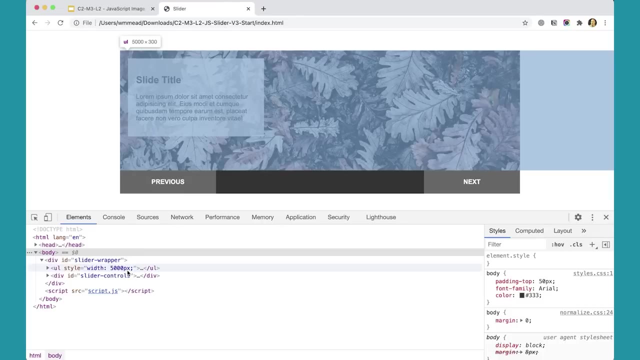 And over here, if I come and look at my slider and refresh this and then click inspect, I should see in here for the unordered list, an actual number of pixels here. UL style width: 5000 pixels, because I've got five slides and there are a thousand pixels wide. 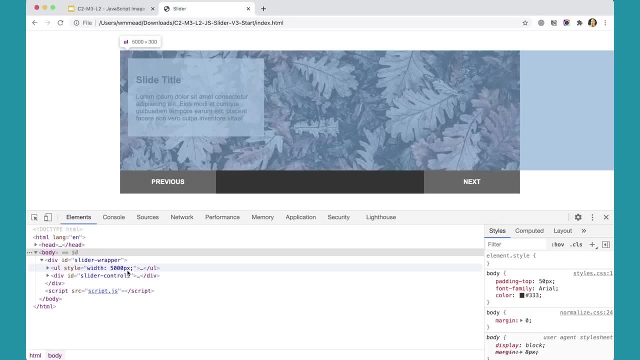 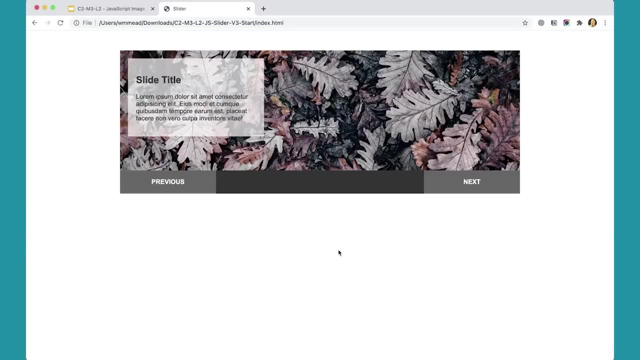 So that's 5000 pixels. So, and the reason why I want to set that here is just in case I add more slides to my slider. I could add more if I wanted to, or remove some if I wanted to, And I want to keep the script as general as possible. 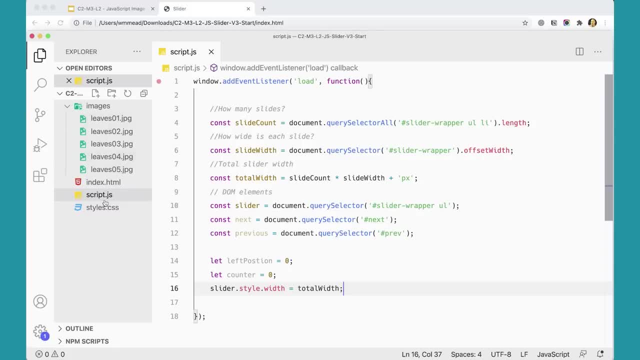 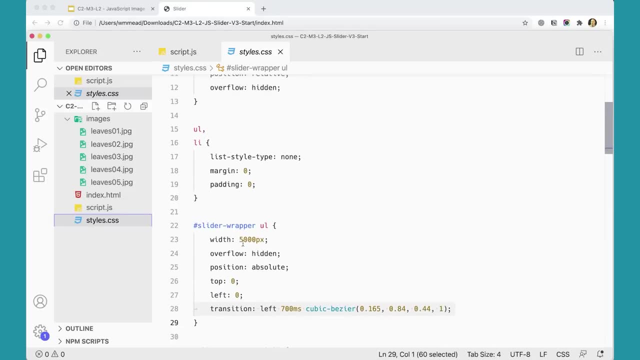 Over in the CSS for this I have in here. I have probably- I think I have- 5000 pixels set here. I have it set here and I could remove that from here if I wanted to now, So I don't really need it here. 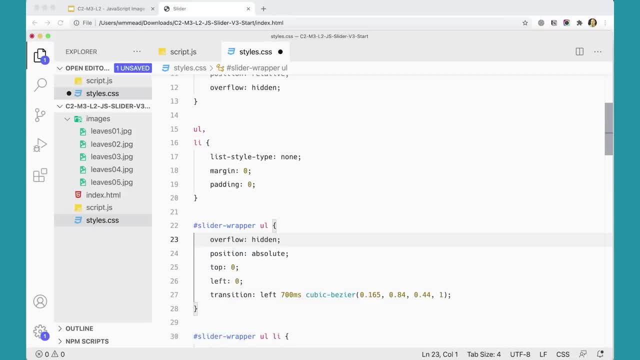 It's getting set on that element manually With an inline style and JavaScript is setting that. So I don't really need it here And really I don't want it here. I want it to be handled by the script, because I want to be able to add or remove elements here. 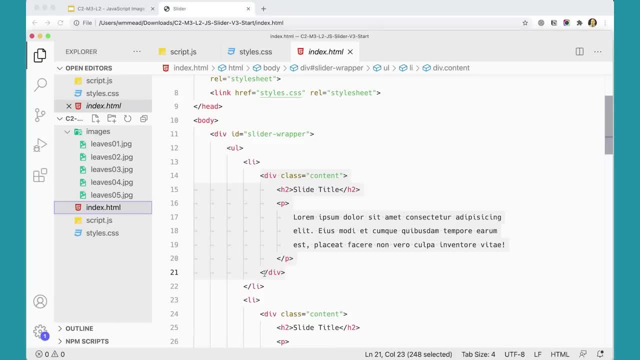 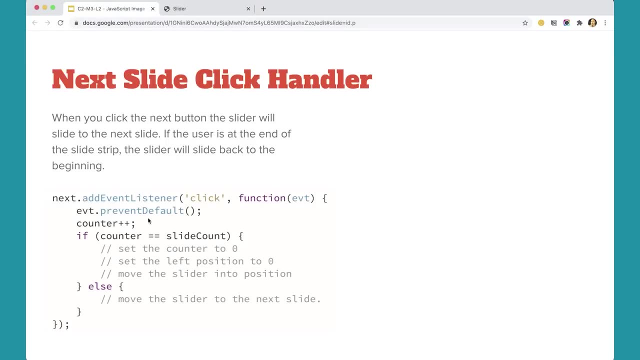 And the script is going to override that anyway, So it's not even really necessary to have it there. So that's kind of a nice thing to pay attention to and to and to realize that I can take that out of there. Okay, So the next thing we need to do is set up our event handler, for when you click the next button. 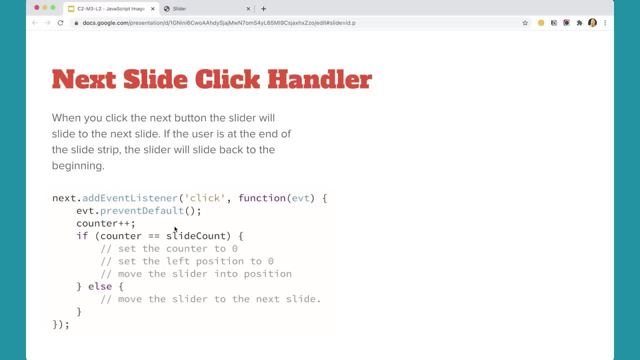 And the first thing we'll do is handle an event. for what happens when you click the link will pass in the event object and prevent default, So you don't get the little hashtag for clicking the next link up in the URL. It's kind of nice. 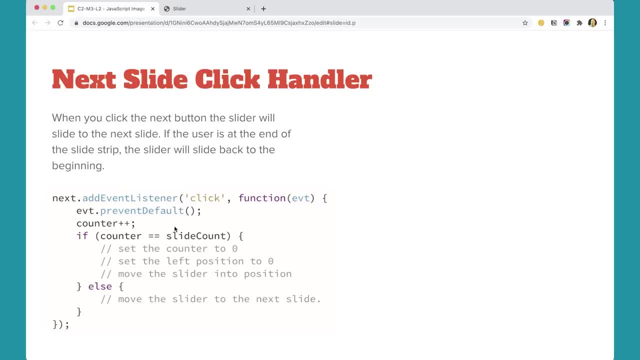 We'll increment the counter, And then we're going to have an if and else, For if the counter is equal to the slide count, in which case we'll set the counter to zero, We'll set the left position is zero And then we'll move the slider into position. 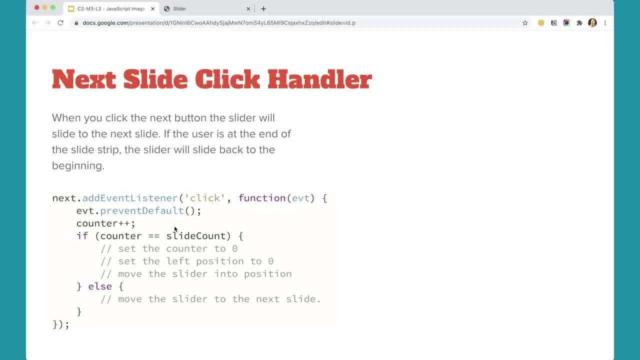 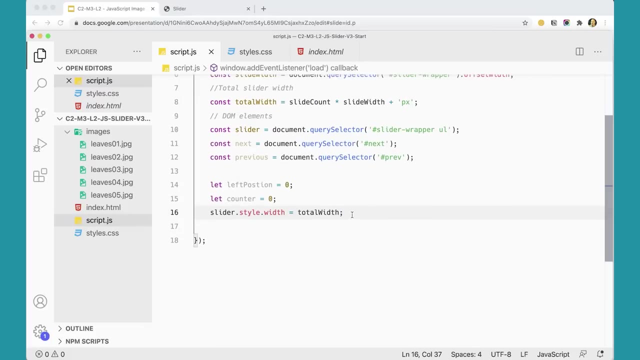 Otherwise we're going to just move the slider to the next slide. So let's go ahead and set up this event listener on our next button. Back to my script. here And now I can just use the handy shortcut Next, Because I know that that is actually going in and getting my from here. 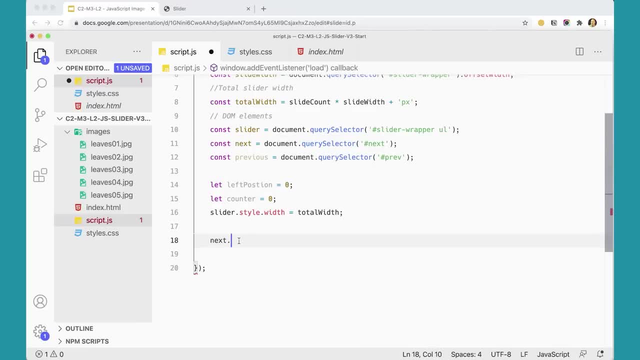 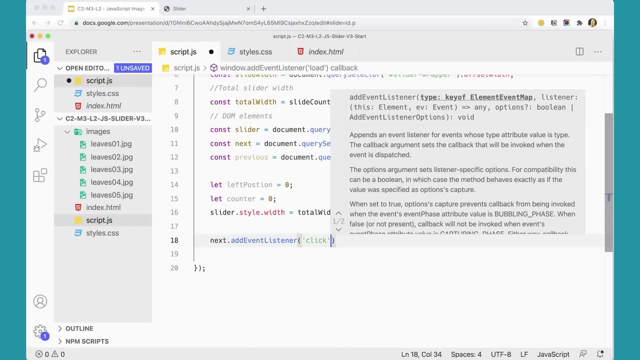 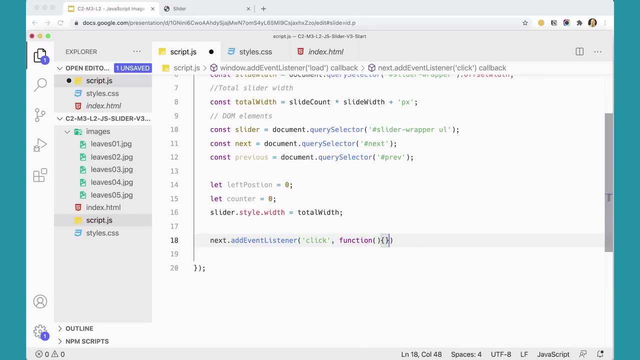 It's going and getting my button pound next. Next Add event. listener. I'm listening for a click And I'm going to run a function When you get a click Like so, And then I'm going to pass in EBT. 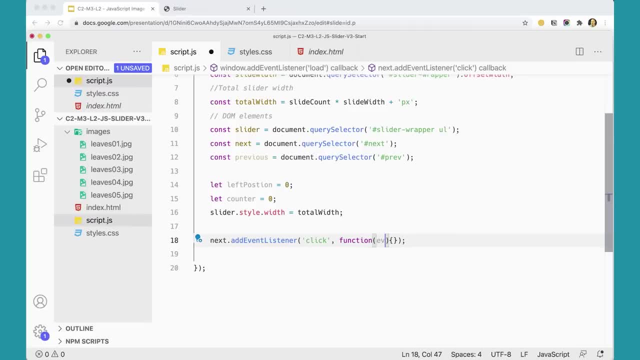 Sometimes people put in event. I usually use event because it's very clear that's what that is. Sometimes people just put in E for event. But E sometimes also stands for error. So I don't want it to stand for error, So I'm going to put EBT. 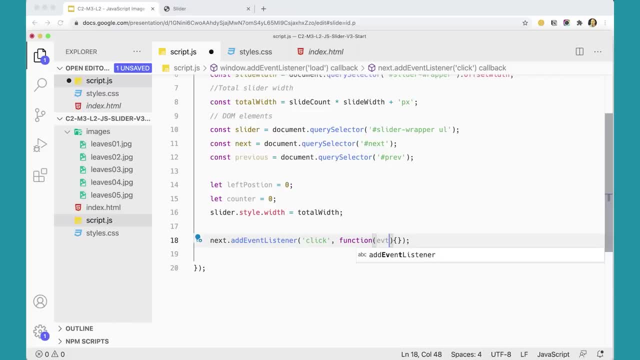 So it's just kind of a nice compromise between the full word event and using the shortcut E, And this is just a variable, So you could put whatever you want. You could make it cheese if you wanted to, or llamas, or chickens or something else. 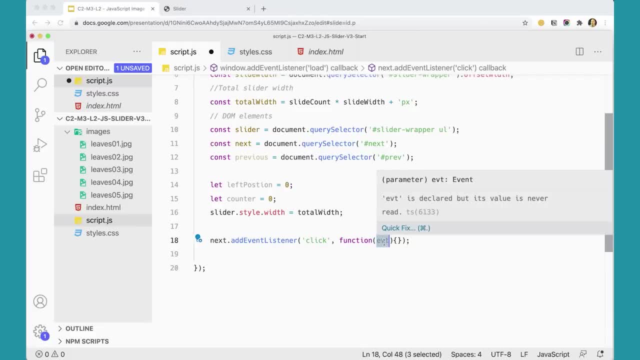 It's just a variable, But it represents that event object that we're passing into this function, The event that happens when you click on this next button here. So down in here we're going to do EBTpreventDefault And that's because these buttons over here 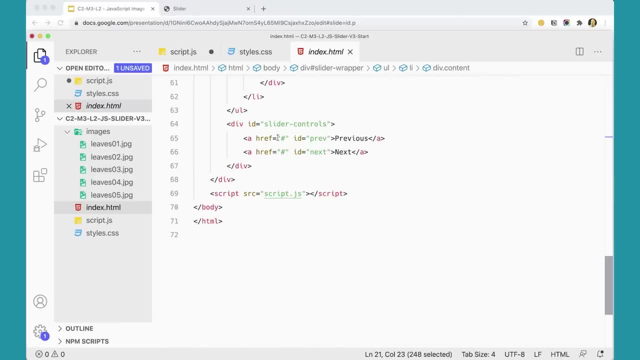 Are really just links, And I don't really like it when this: If you click on the link without that, Then this pound sign ends up in the URL This hash, And I don't really like that. So the eventpreventDefault keeps that from happening. 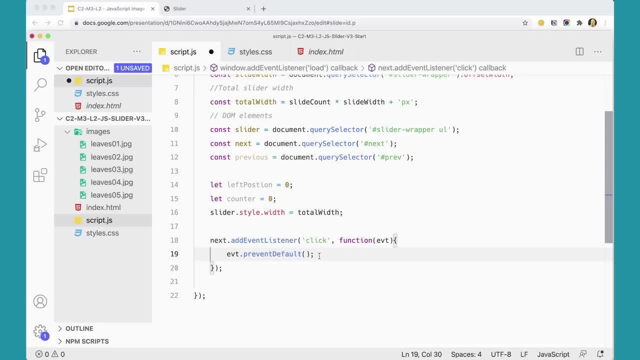 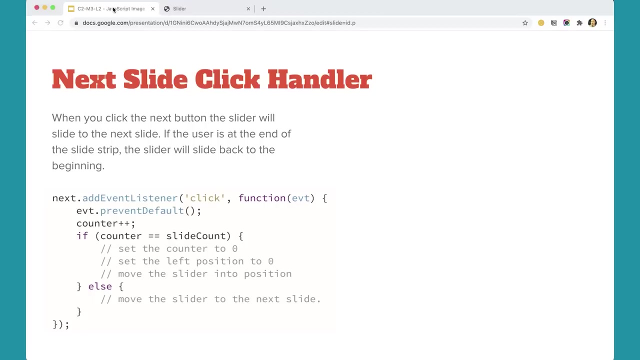 EBTpreventDefault Passing in that thing. Okay, Then we're going to have an if statement, If We'll handle what happens If The If the counter Has gotten to the end of my End of the line And an else. 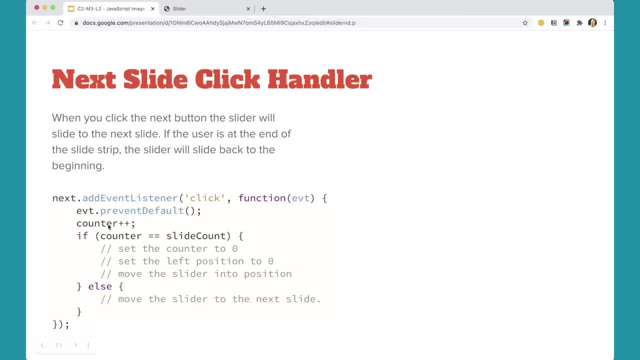 And again, what we're going to put in here is: We also need to increment the counter. Counter is the same as slide. count Equals equals The same as. Read that as the same as. So don't forget, we need to increment the counter. 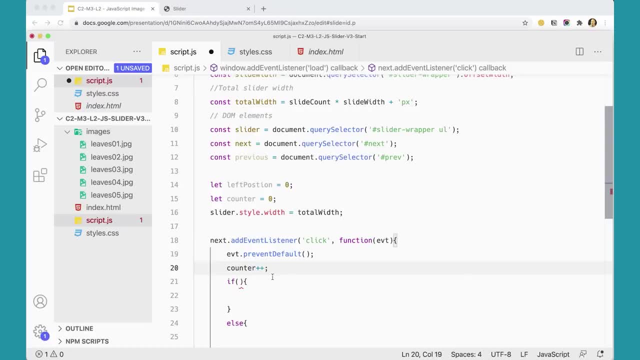 Counter Plus plus The same as Counter equals counter plus one. Just a nice little shortcut there. And then If Counter Is the same as slide count, Then we're going to do something in here, And then we've got an else in there. 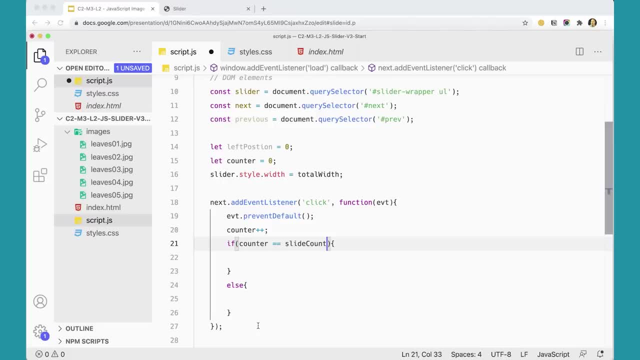 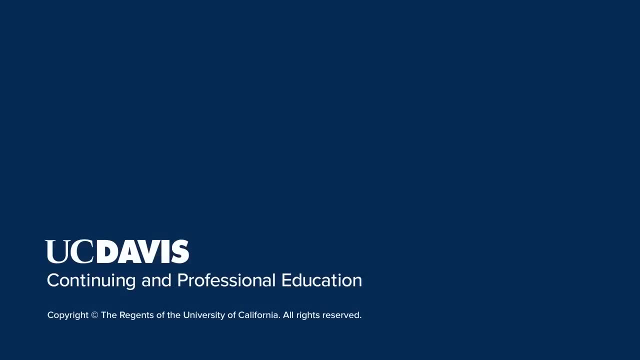 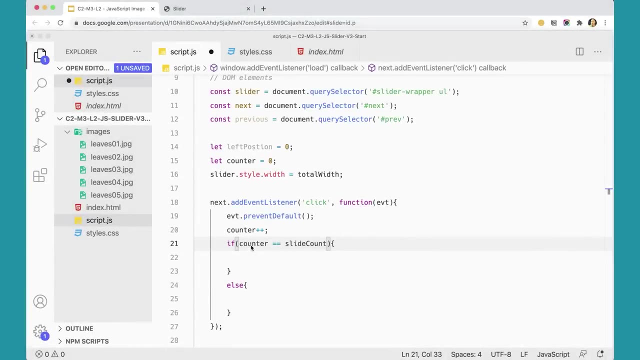 And then we'll pick up The rest of this Next event listener In the next video. If we've reached the end of our strip And the counter is the same as the slide count, Then the first thing I want to do- 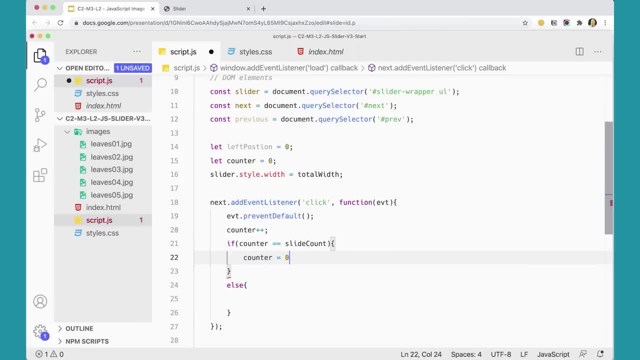 Is set that counter back to zero, Then I want to set this variable left position And make sure it's set to zero Left position. It was set to zero initially. I just want to make sure it gets set To zero again. 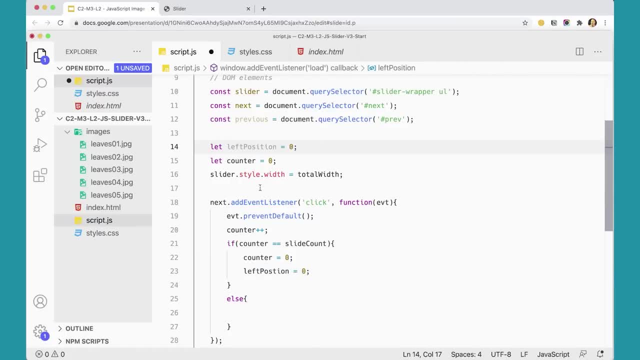 And of course I misspelled position there. Left position. There we go. I'm going to make sure that gets set to zero And then I'm going to take my slider Style Left And set it equal to left position. 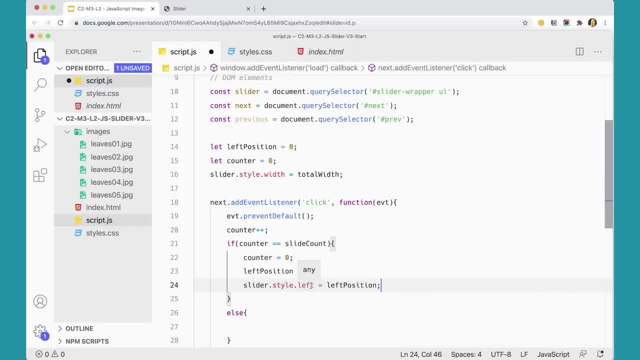 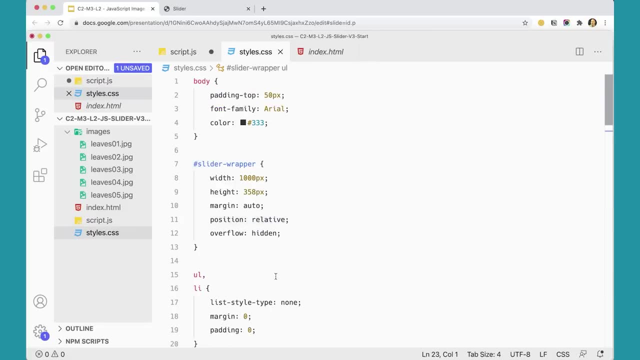 And that will put it into the correct position on the page. Now remember, over here on the styles, When we talk about slider, We're talking about This unordered list here And it has the transition on it. So that's going to take care of the animation. 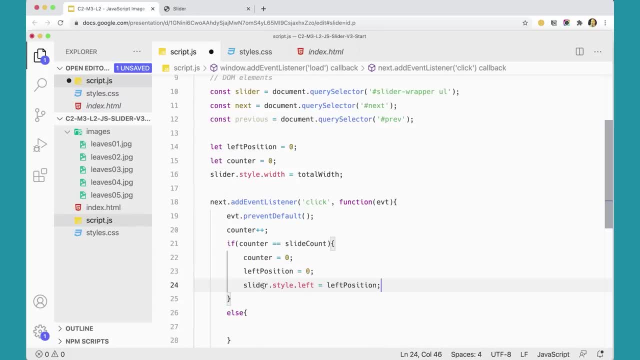 So I don't have to do the animation over here. All I have to do is set that position left And CSS will handle the animation. So that's one thing. that's different Between the JavaScript version And the jQuery version. In the jQuery version, 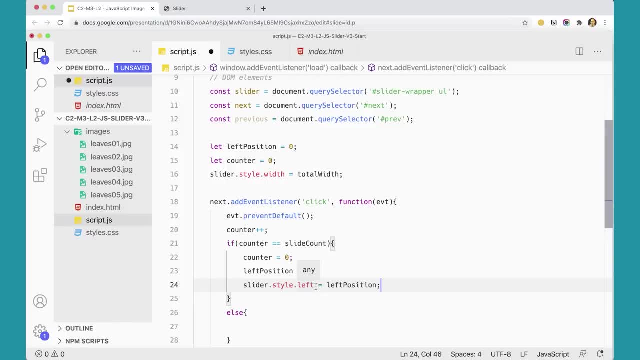 We're using the jQuery animate method, Which is using their built in effects library For doing the animation. Here we're just setting the CSS position Of the CSS property of left To left position, Which in this case is zero, And then we let CSS handle the animation. 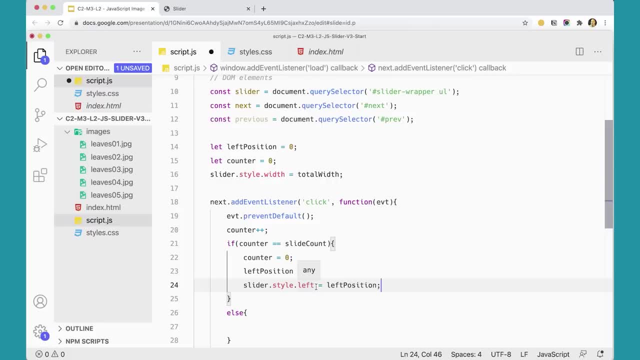 And because CSS uses the GPU Instead of the CPU, It's kind of nice and buttery smooth And it will work well on older devices That don't have a faster processor. On a newer device, The jQuery will work fine, But older devices- 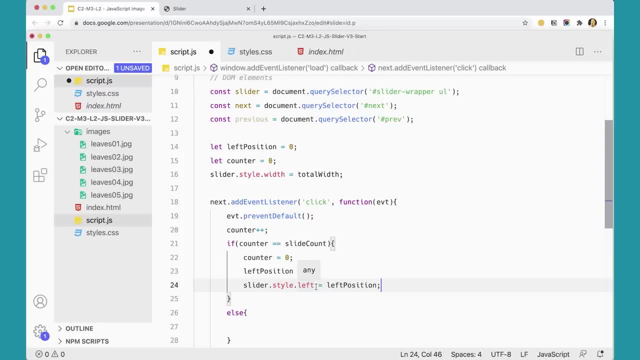 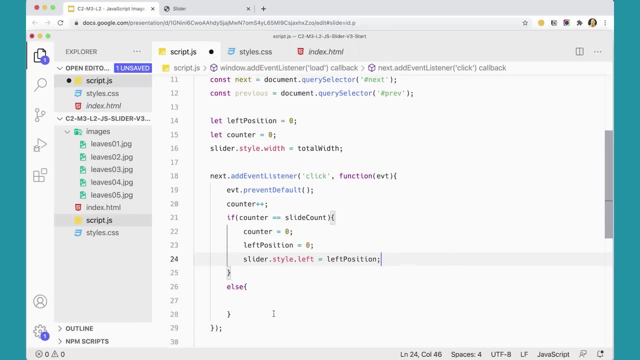 The CSS in particular Will work a little bit better And be a little bit smoother, But I think it's even smoother on newer devices, Honestly. So that takes care of the if statement here For the, else We need to increment the slide forward. 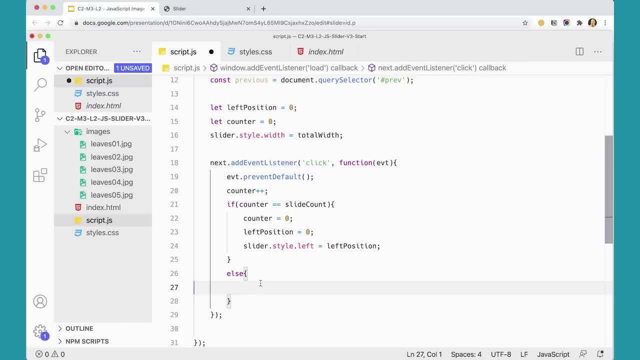 If we're not at the end, We're just going to move that slide forward. So I'm going to set left position here. Left position Now spelled properly. I'm going to set it equal to. I'm going to use a pair of tick marks. 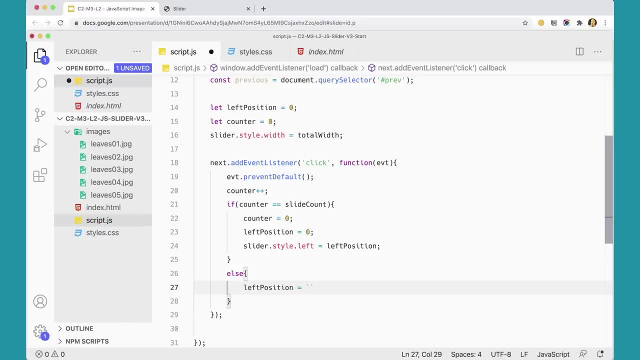 And I'm going to set it to a negative number, And what I want it to go to Is I want it to go to Whatever the counter is. Times The slide width, So I'm going to put in your dollar sign. 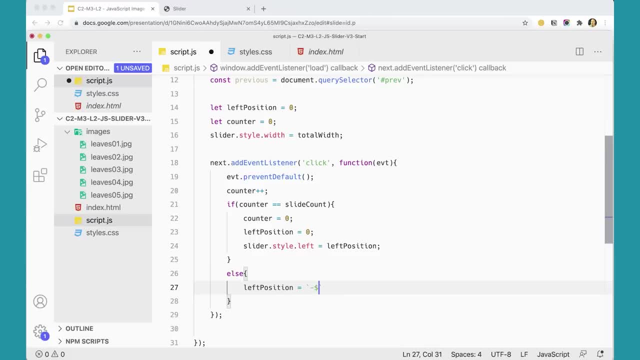 Curly brace Counter. So if I'm clicking it the first time, That counter is going to go from zero to one. So that's going to be one. And then I want to multiply it. Times: Slide width: That's going to be one. 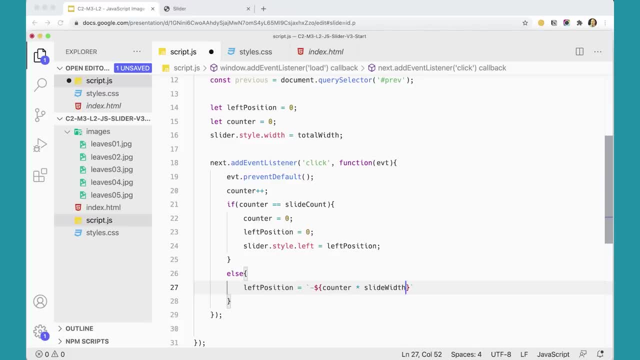 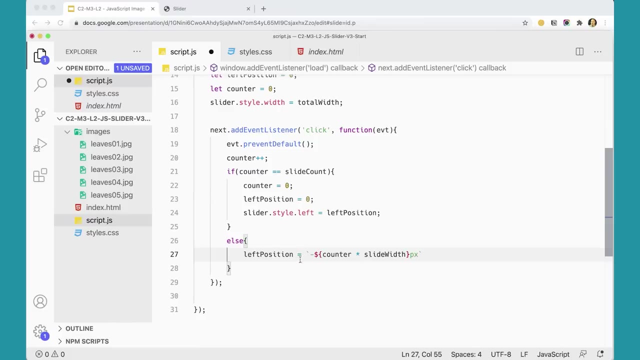 And of course, I want to add a PX in here. I believe the slide width doesn't have the PX Now, it's just the width. So I need the PX in there, So that sets that left position there And then, And then I just need this: 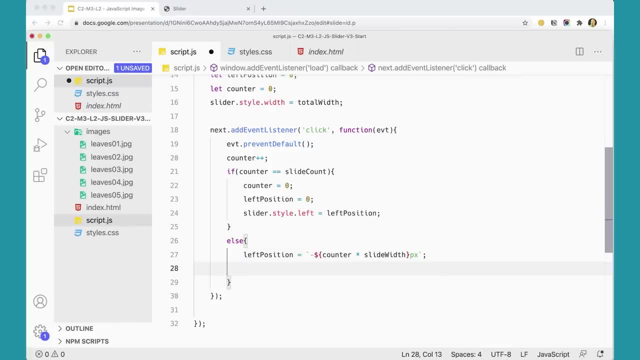 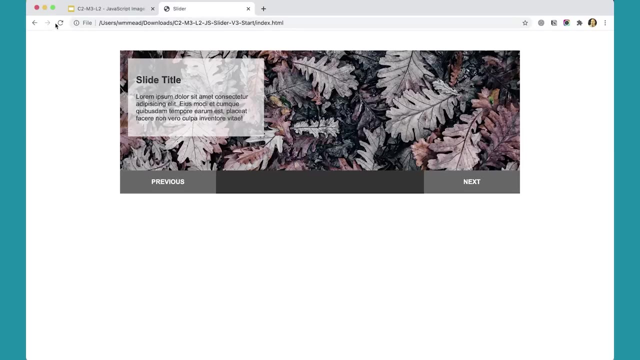 Same thing. I'm setting that, setting that left Property to what the left position should be And that should, in theory, work. Let's go check it out, Refresh, See if I did it right And notice it's nice and smooth. 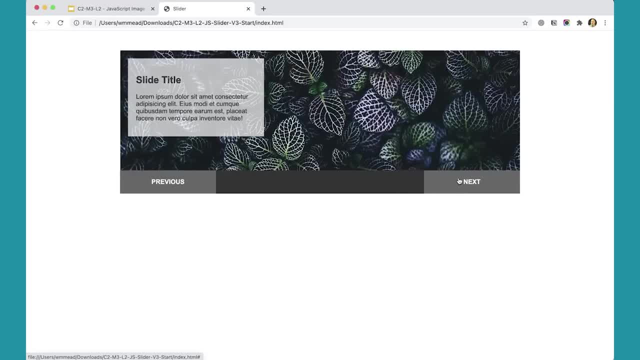 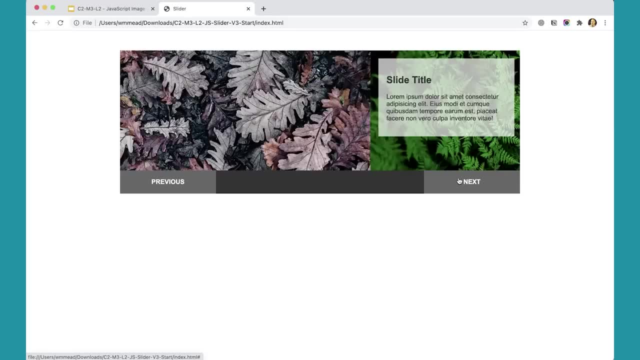 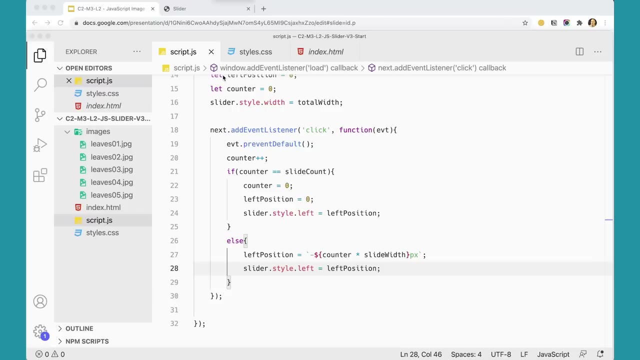 The animation. When I get to the end, it goes back to the beginning. We have a script that's working And this is perfectly fine the way it is, But it could be simplified a little bit. If we look at this, You'll notice this line. 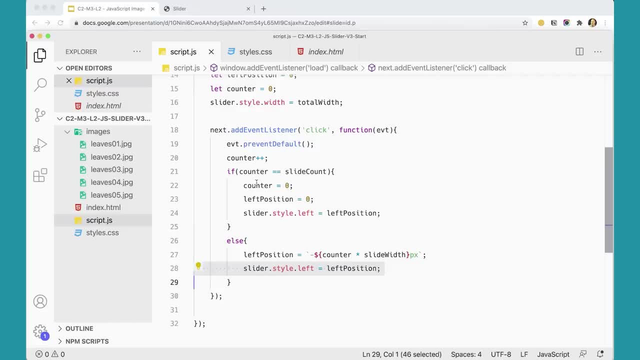 Is the same as this line And really If I set the counter to zero, I don't need to explicitly Set left position to zero, Because this will do the same thing. So if I get set counter to zero, Zero times slide width: PX. 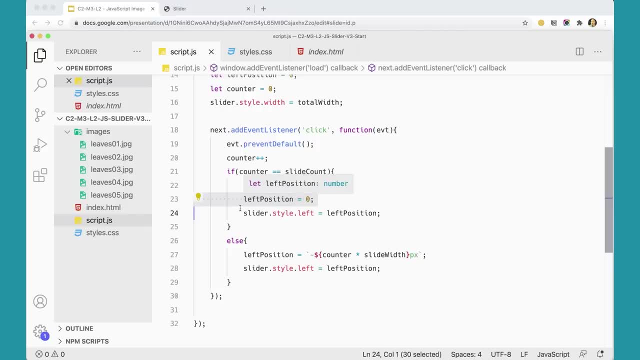 Is going to be zero, So I don't really need this line either. So in fact, My if statement could get much shorter. It could just be If Counter is zero. Counter is the same as slide count Set counter to zero. 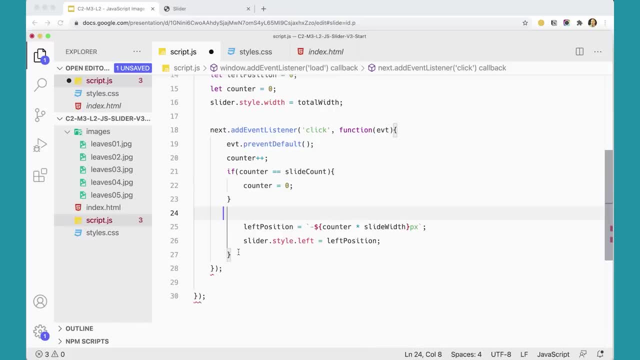 And then I don't really need an else, Because this is going to happen, no matter what. Like so, And you could. You know, If you wanted to make the script even Kind of shorter, You could put these on one line. 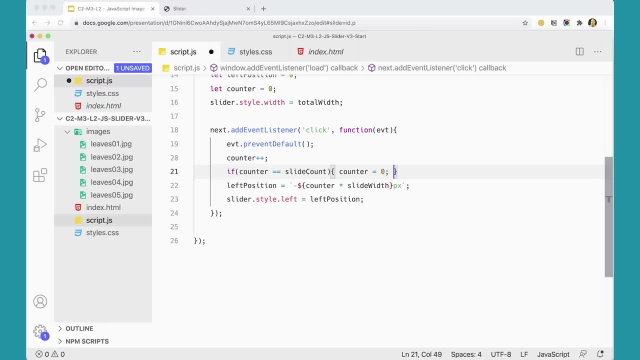 I think Visual Studio Code is going to Scream at me when I try to do this And put those back on two lines As soon as I save this. But You could even just put this all in one line, So it makes this. 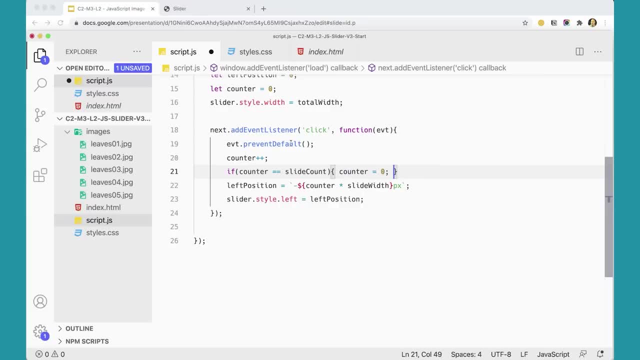 Really nice and short and compact. We're Setting the The event Prevent default. We increment the counter. If the counter is the same as slide count, We set the counter to zero And then we set the left position to Whatever the counter is. 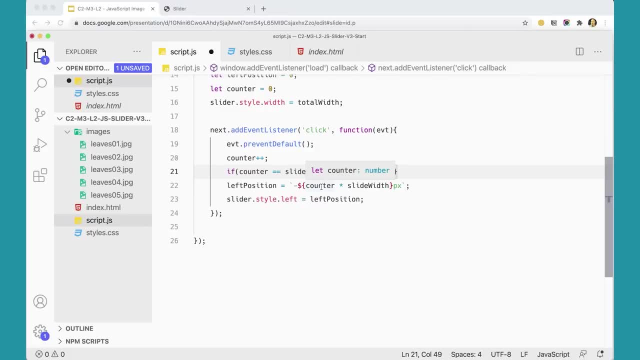 Times the slide width. If it's zero, Then it's going to be zero, And that's fine. If it's one, Then it's going to be One times slide width: 1000 pixels Minus 1000 pixels. 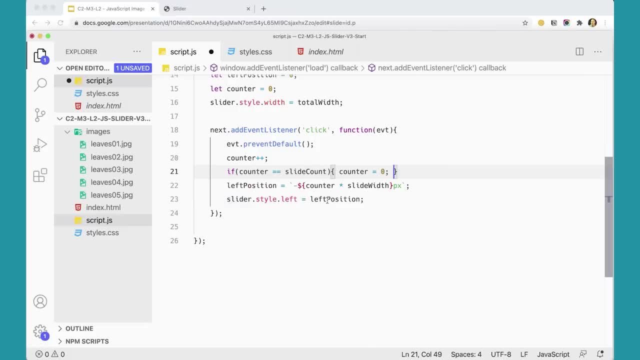 So on and so forth. And then we set The slider style left to left position And let the CSS do the animation, Save that And Come over here And you'll notice it should work exactly the same way. I click next. 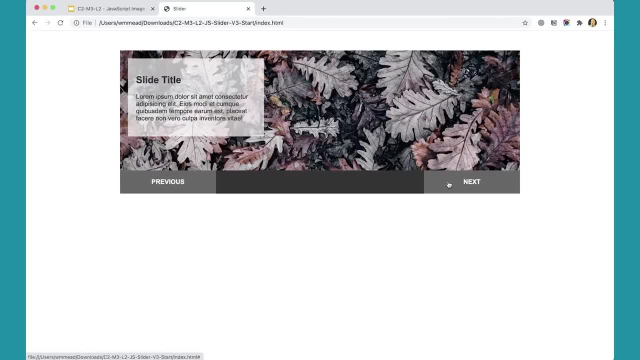 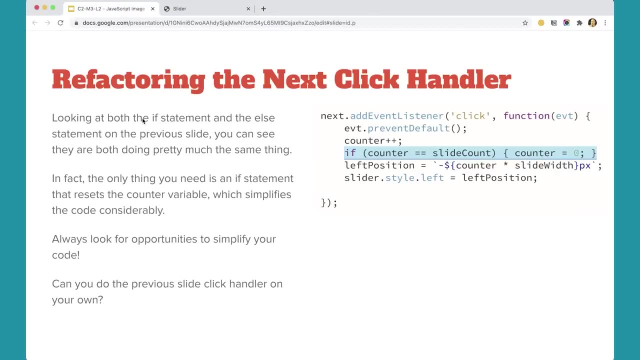 It's going all the way to the end And then back to the beginning. So that's great. Okay, great. Now We've got that in place And that's all working And that's awesome. So Your chore Is to do the previous. 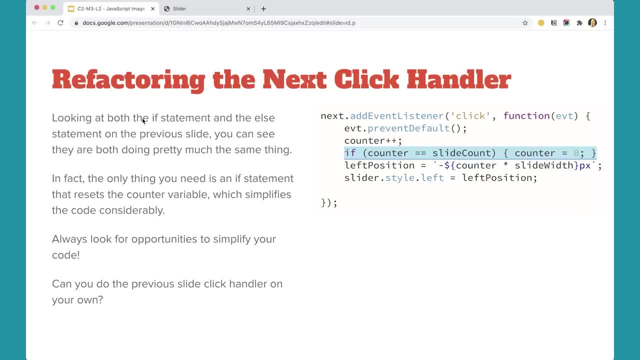 Event listener, And this one's not as hard As the, The jQuery one, But It's very similar to what we have here, Except we're using the Previous link And we're decrementing the counter, But Other than that, 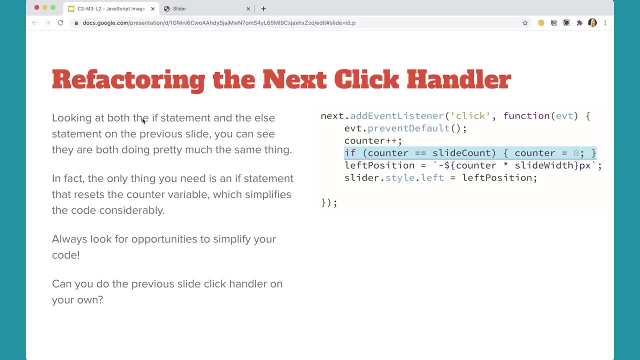 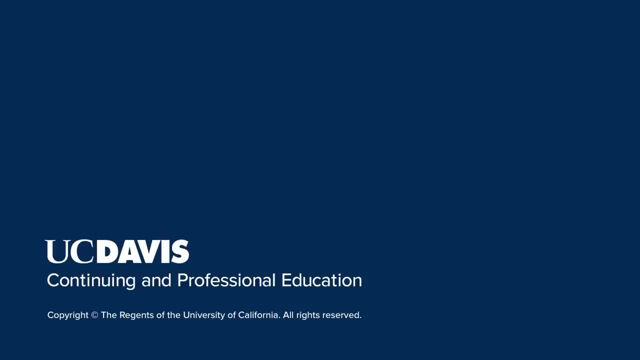 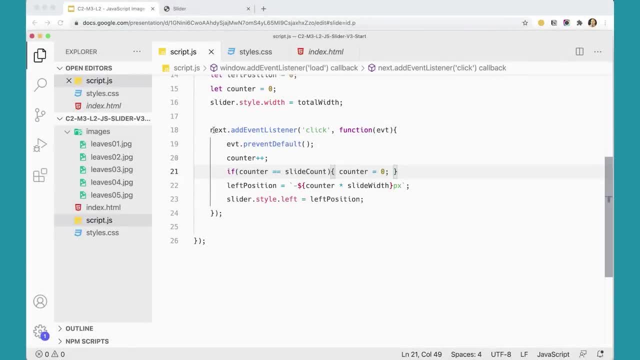 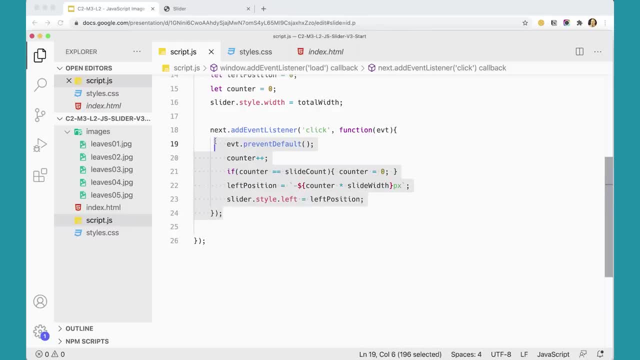 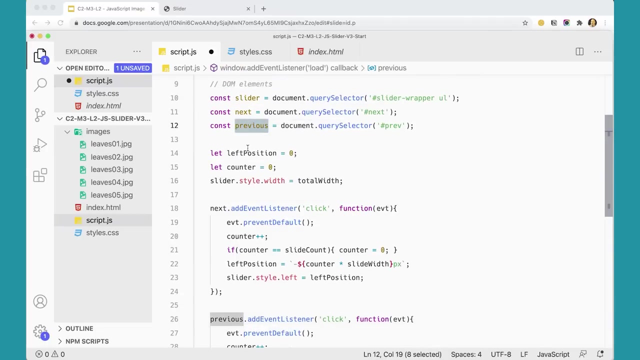 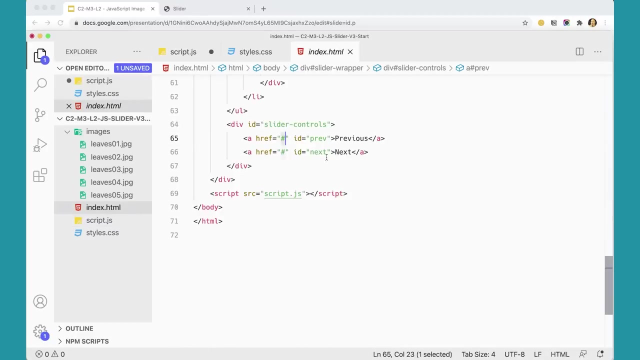 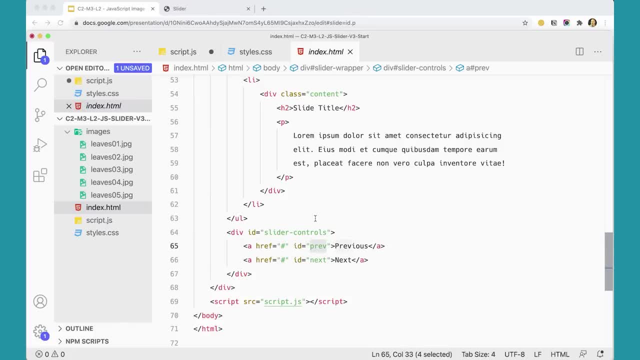 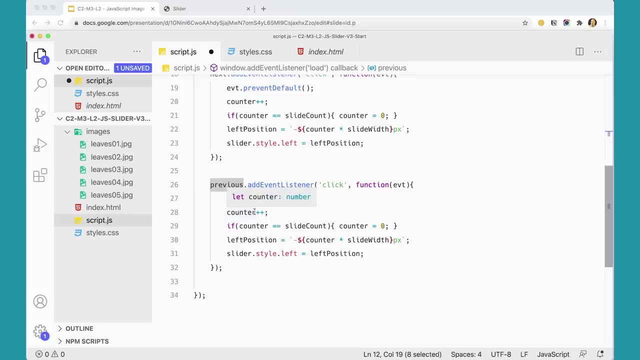 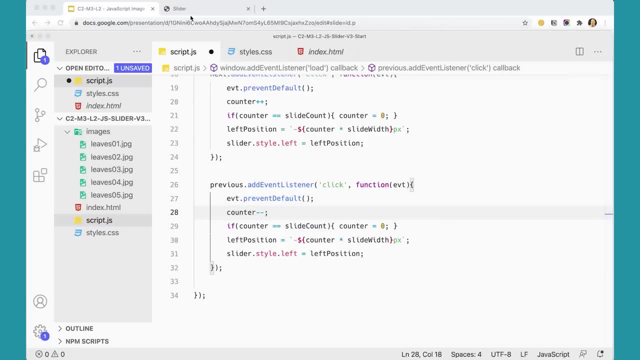 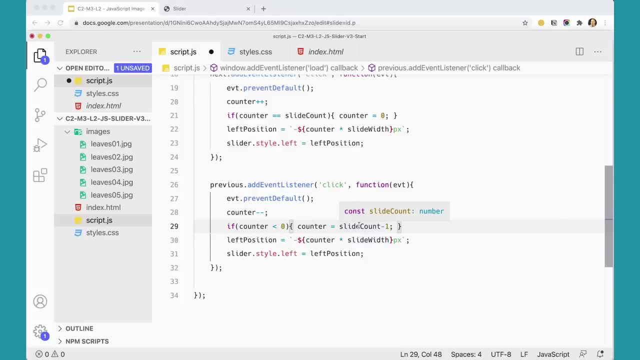 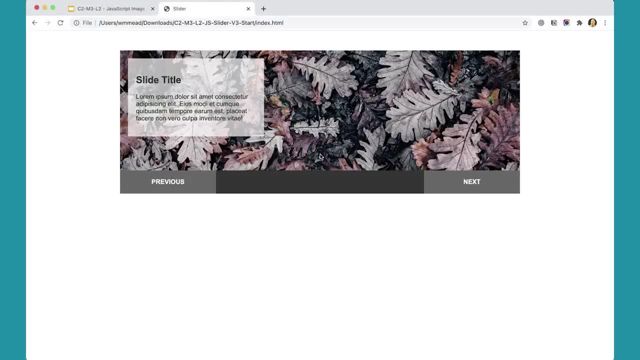 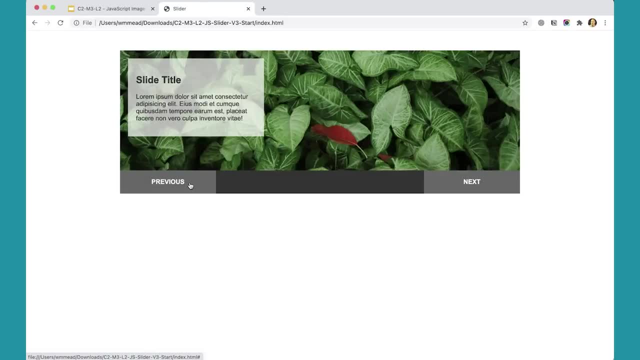 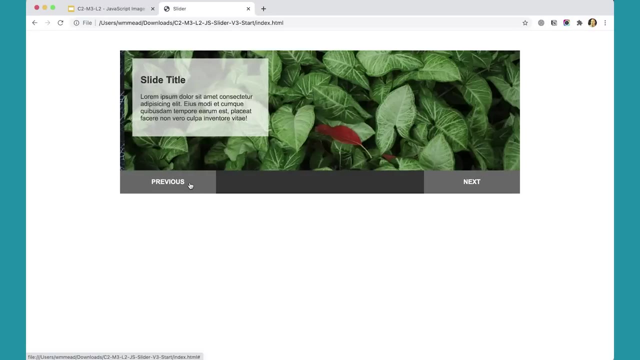 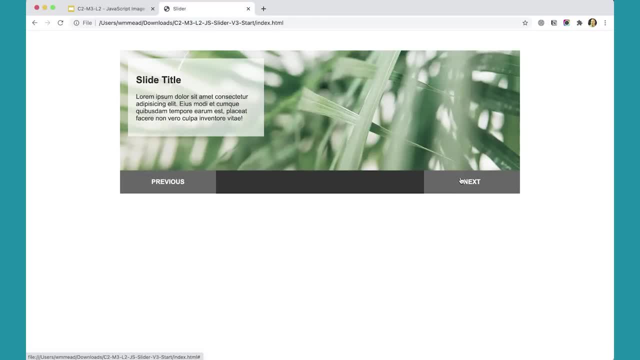 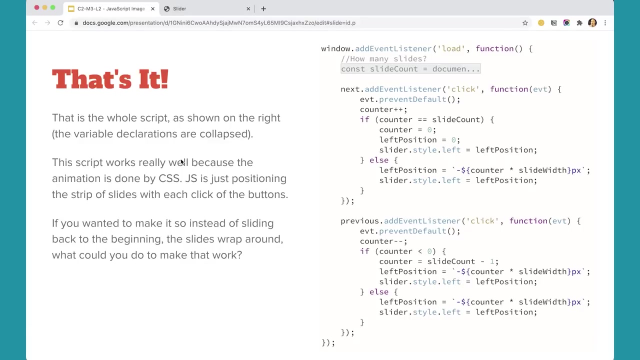 So now I have a slider that is working, that's going from slide to slide and it's moving the strip along back and forth through here. That's it. You've completed this project. Here on this slide, you can see the full script with everything in it that we needed. 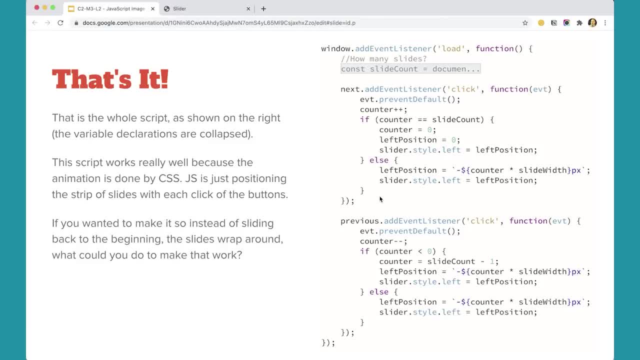 You can see I left the else statements in here. I don't really need these. This is actually the longer version of it, But that's pretty cool. We've got a full version of that script and you could use this on your websites. 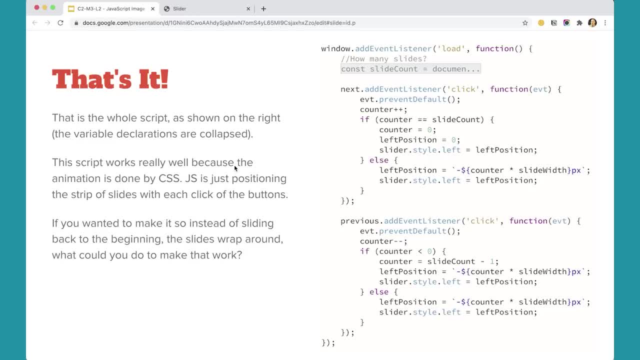 and compare this to what we did with the jQuery versions. Now, if you want a challenge, try to make the version of the JavaScript slider work where these slides don't Go all the way back to the beginning or go all the way back to the end. when you get to the end, 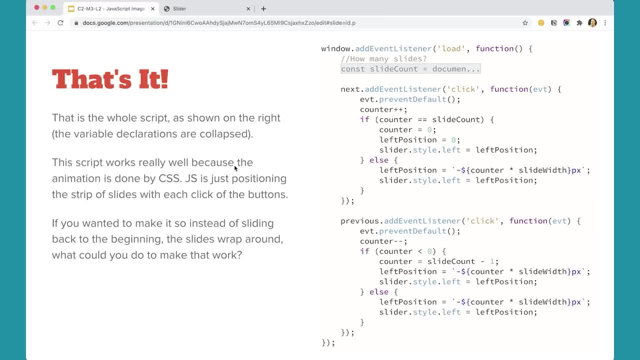 Make it so that it wraps around, Do the second version of the jQuery script, but just with JavaScript, And hopefully that will work. Okay, And with all of that, hopefully this is a great project for you and you've learned a lot about JavaScript along the way. 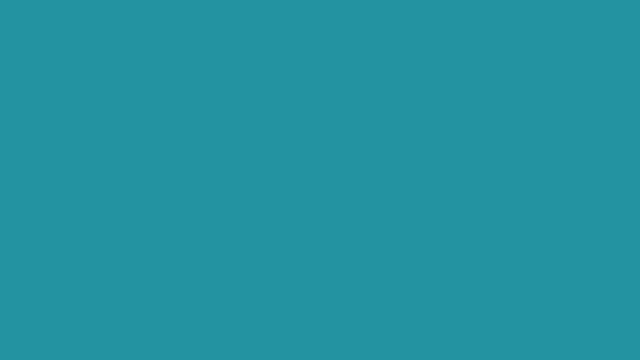 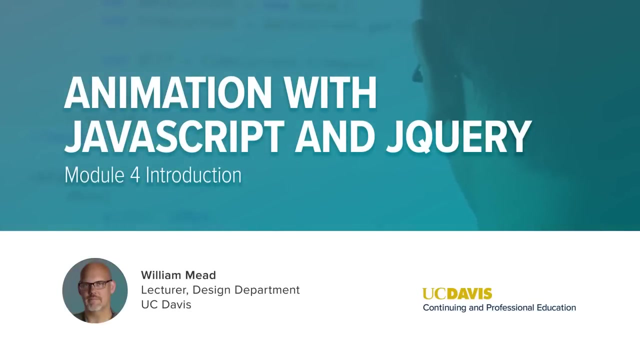 Thank you so much for joining us today and I hope you have a great rest of your day. I'll see you next time on JavaScript in jQuery. Bye-bye, Bye-bye. Hello. You've made it to the fourth module in our second course on JavaScript in jQuery. 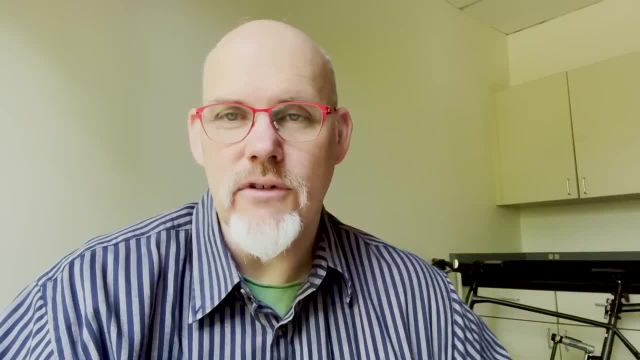 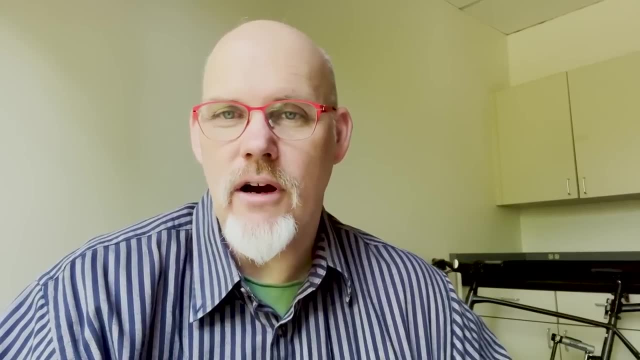 Congratulations. You've learned a lot of JavaScript and a lot of useful jQuery for all of your interactive projects. I think it's a lot of fun and I hope you've enjoyed the ride so far. In this module, we're going to get into a little bit more about JavaScript. and we're going to get into a little bit more about JavaScript. and we're going to get into a little bit more about JavaScript. 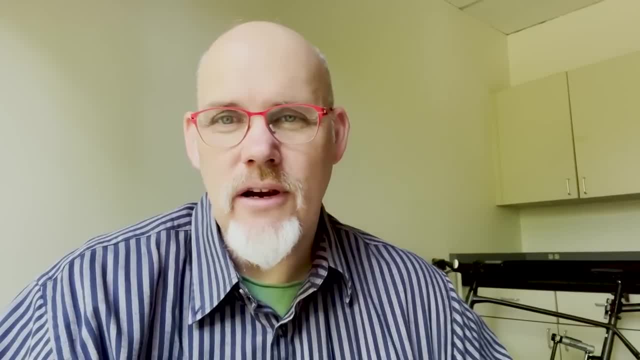 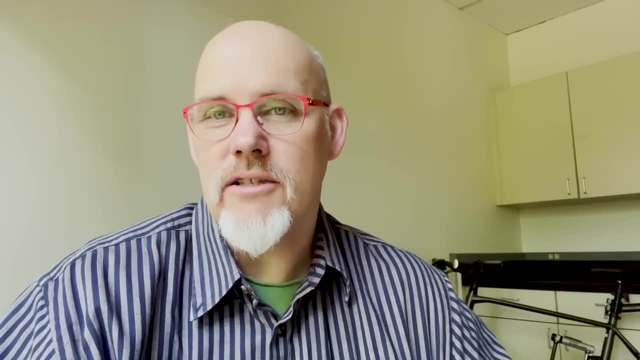 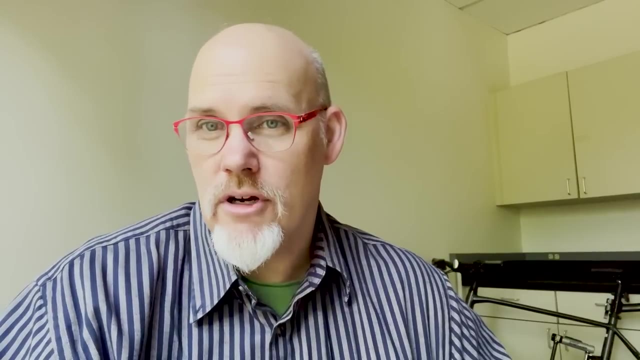 In this module, we're going to get into timers and recursion, and these are very useful tools that will open up a whole world of possibilities for JavaScript in jQuery and for your interactive projects. So break out your code editor and your web browser and let's get started on learning about timers and recursion in JavaScript in jQuery. 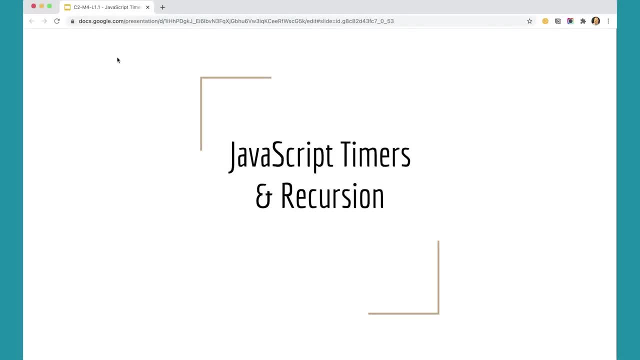 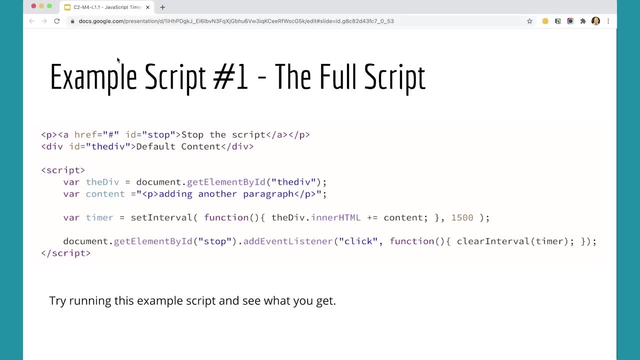 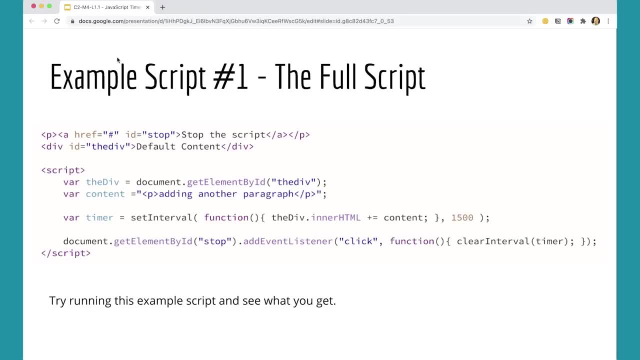 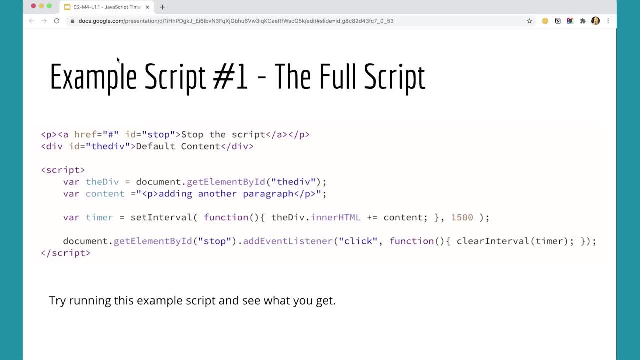 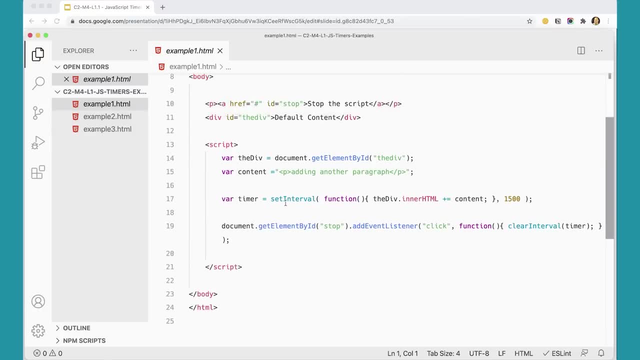 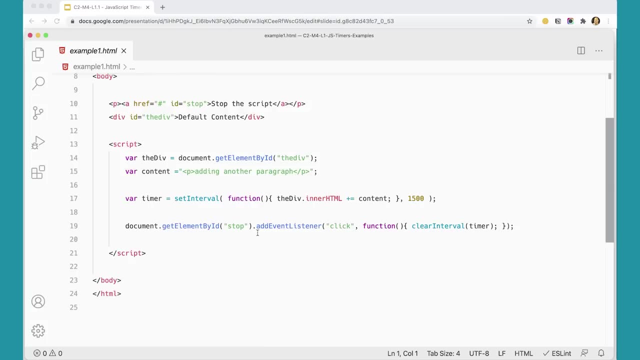 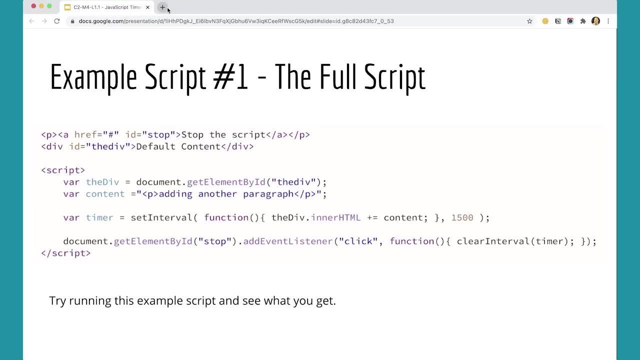 here i'm looking at example one, and this is the script here. it's very, it's a very short script. i'm going to close my explorer here, just so you can just see this line without it wrapping. but, um, best thing to do is to actually see the script run. so let's, i'm going to come over here and just 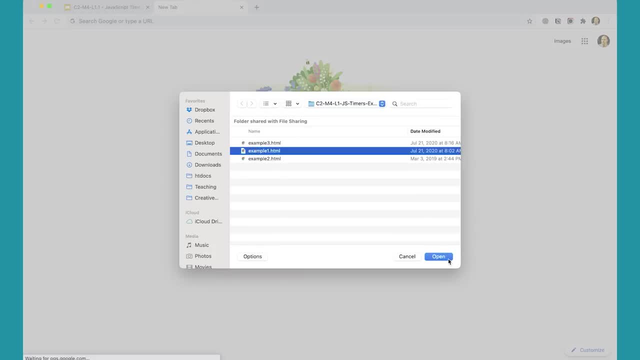 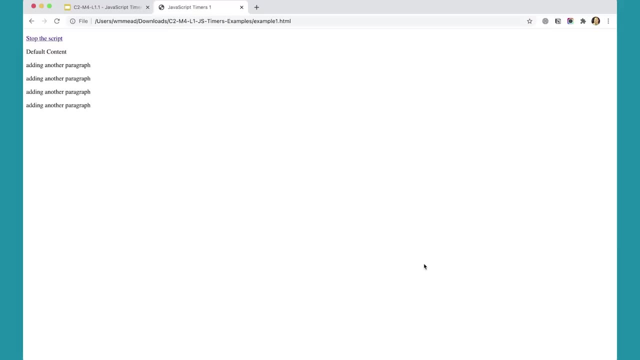 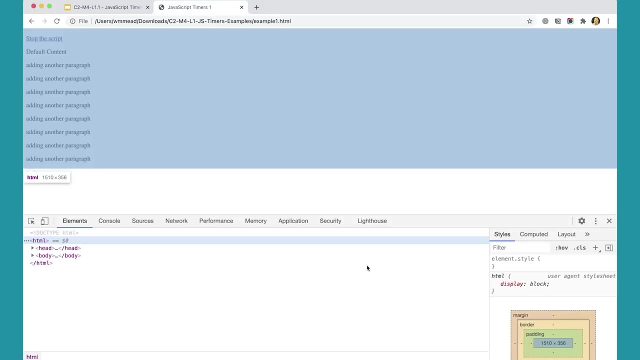 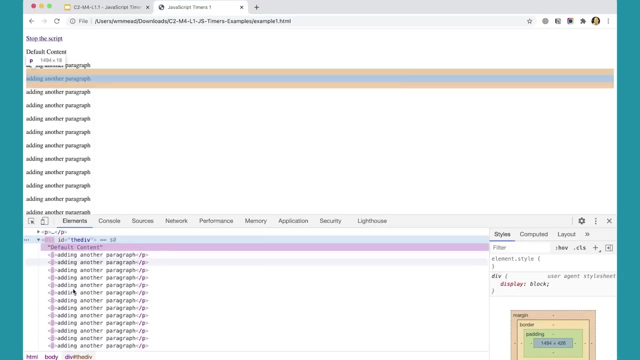 open the example one script here and you'll notice that after a certain amount of time the script starts adding paragraphs to this web page and if i view the inspector and look at the body here and my div, you can see that this div it's adding another paragraph. 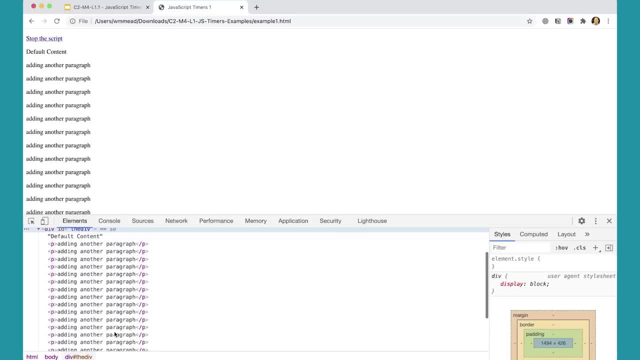 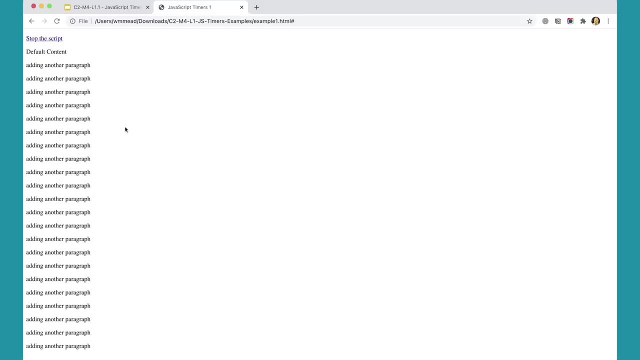 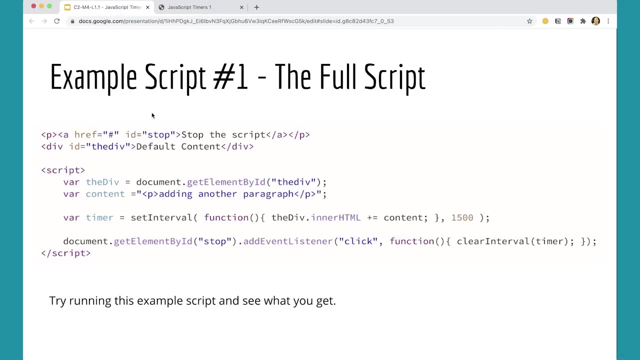 every second and a half it adds another paragraph. if i want to stop the script, i can click the link stop the script and it will stop adding paragraphs. so let's deconstruct how this works just a little bit here. that's the full script and essentially there are two functions. 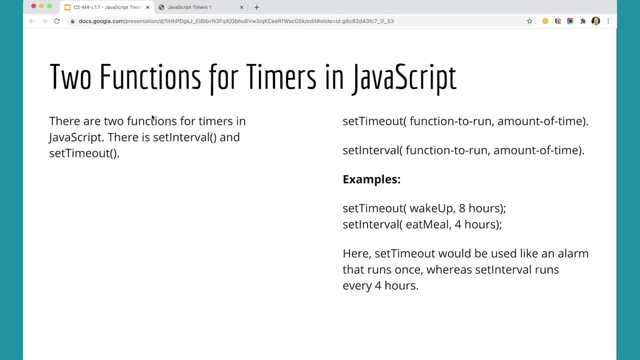 in javascript that allow us to set timers. one is set timeout and the other one is set interval. each of these functions takes a callback function and an amount of time. so for set timeout or for set interval, you would run a function and then you'd put a comma and then the amount of time. 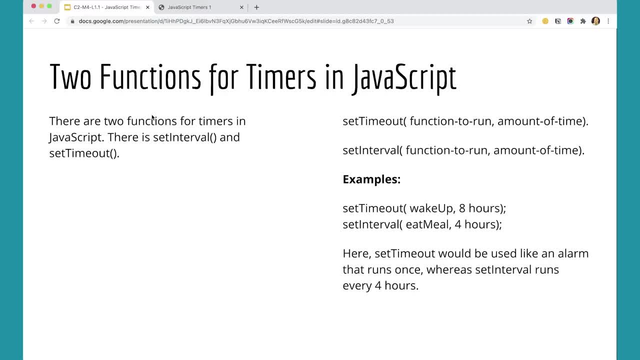 that you want to have a lapse before it runs or on the timeout, the interval. so for example, down here i have set time out wake up, so it would run this function: wake up after eight hours. or set interval: eat meal after four hour. every four hours i'm gonna eat a. 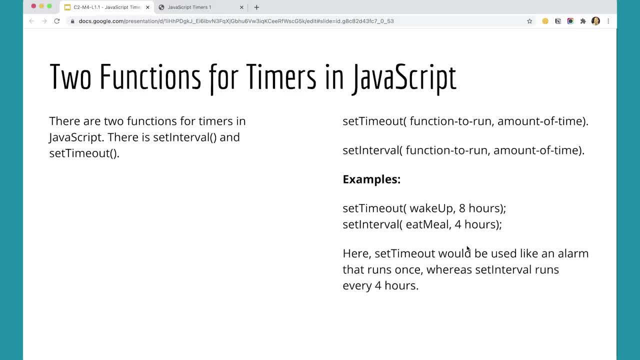 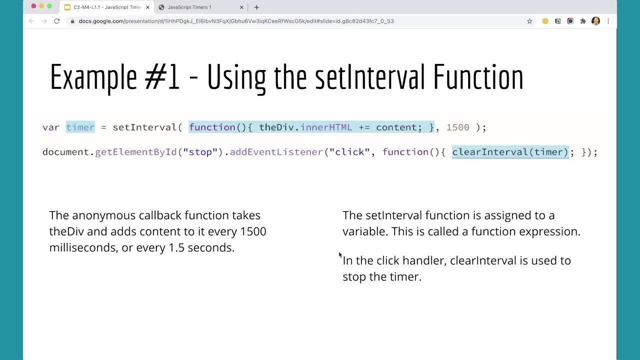 meal, something like that. um, now you can't pass in eight hours and four hours. you pass in a number that represents milliseconds, but, um, but it's that basic idea. so let's take a look at our script here we have a timer that is a variable and it's assigned the set interval function and if you'll, 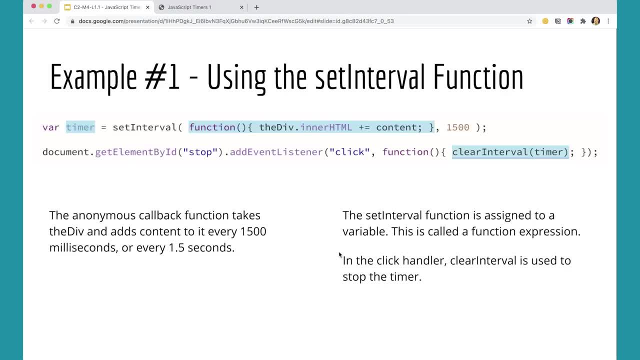 remember this is called a function expression because in javascript, javascript is a is treats functions as first class citizens within javascript. so you can assign a function to a variable. just the same way you could assign a string to a variable, or a number to a variable or anything else to a variable, any other piece of data. you can assign a function to a variable. 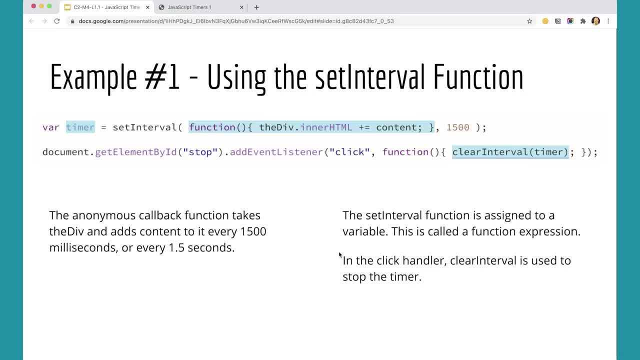 and that's one of the things that's very powerful about javascript, and it allows us to assign functions to variables. so i've assigned the set interval method to the variable timer and then the set interval method has a function in it and the function simply says: take the div dot inner html. 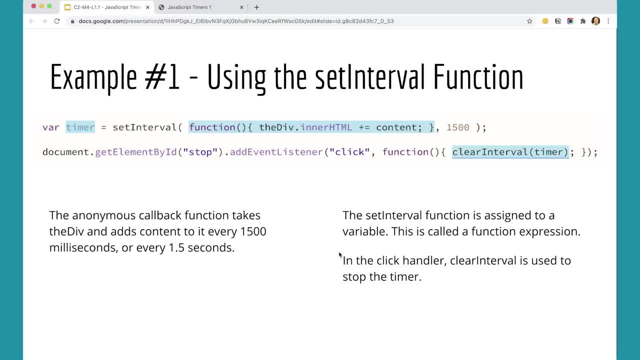 and plus equal the constant, and so we'll take some content and add it into the div, and then we'll do that every 1500 milliseconds or every second and a half, and so that's how this is. adding the adding the content onto the page is that timer loads and set interval immediately starts running. 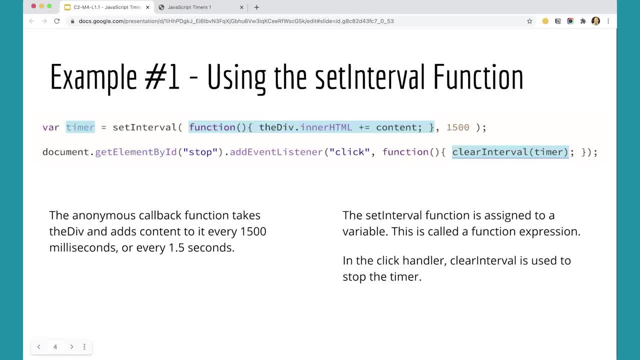 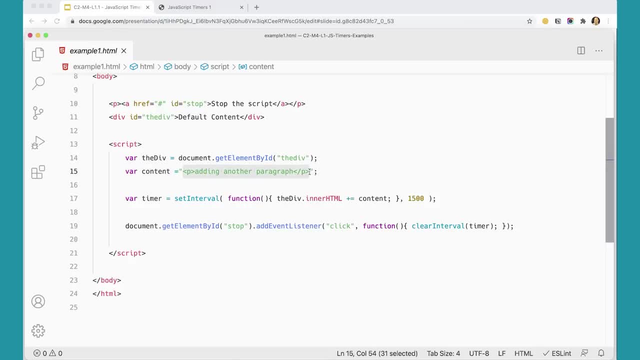 and starts doing its thing and adding this content in the page. let's go look at the script again in the actual file over here. so i have the content here which is adding another paragraph- it's just a string here- and then set interval runs and it says: take this div, the div. get element by id, the. 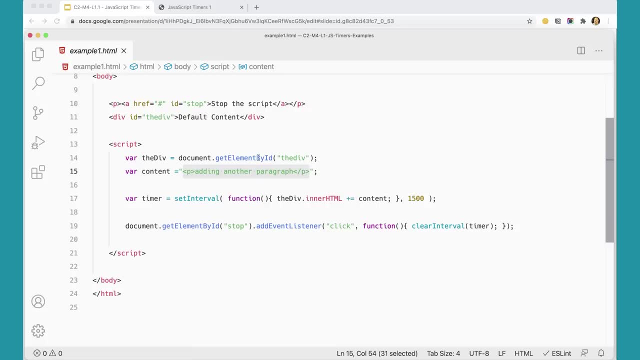 div, which is this div here. it's got some default content and it's going to set its inner html to content. so in a second and a half the content is going to get switched to a paragraph and it's going to add that to the name. so we're going to go ahead and add this and we're going to enter this to our div of two, which is a javascript in a dot Subt rack drop. 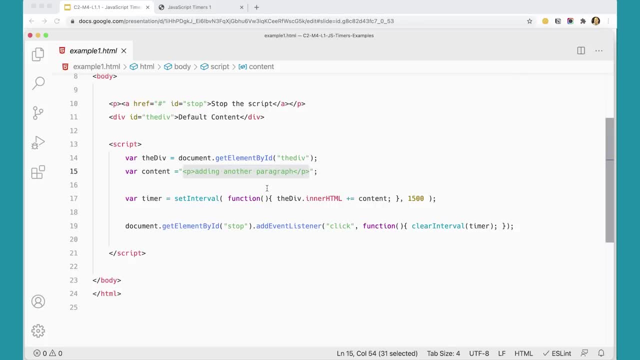 It's going to set the inner HTML to that content And then in another second and a half. then what's going to happen is the content plus equals is going to take the content and add it again. So now there's two paragraphs in the content. 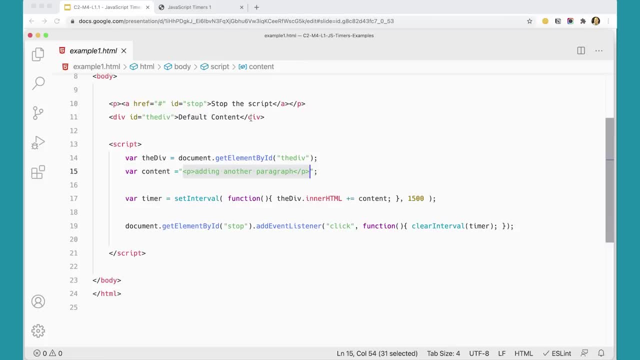 and it's going to change the inner HTML and div to having the two paragraphs. So the two paragraphs are on the page and so on and so forth, until the page is completely full with the paragraphs. We'll talk about the clear interval method in the next video. 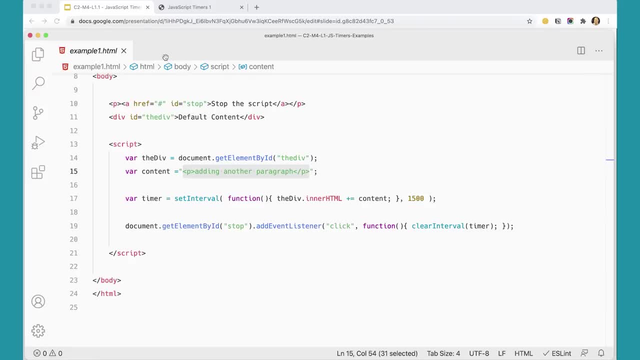 We're looking at the first example in our timers and recursion examples here And we've already talked about how this example is using set interval to keep adding content into the div and then adding those paragraphs onto the page, And we have to remember that the set interval 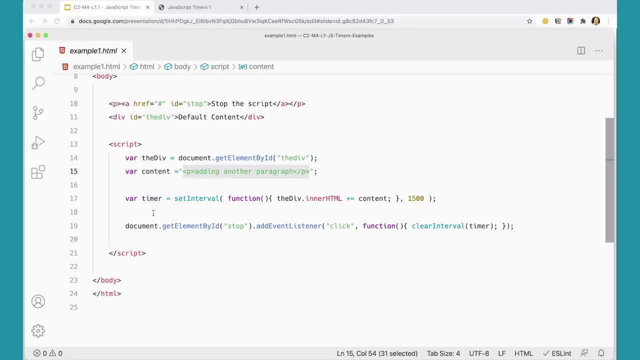 is assigned to this variable timer And down here I have an event listener that when you click this button, stop ID, stop document, get element by ID: stop. it's got an event listener. When you click on it it runs a function. 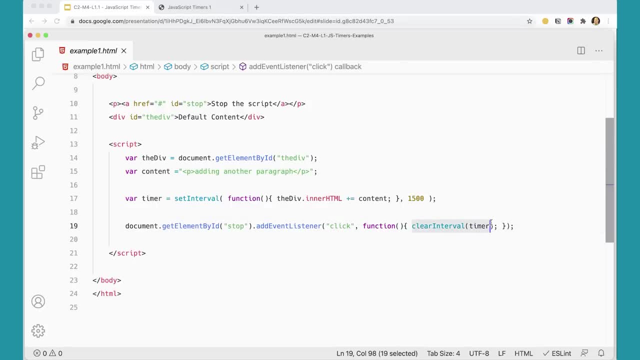 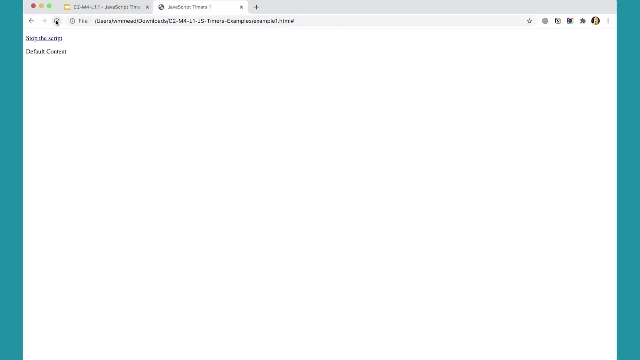 And the function runs this method: clear interval and I'm passing in timer. Timer holds the set interval thing here, So that's what allows me to stop the script So up here. when I refresh my page it'll automatically start adding content into that div. 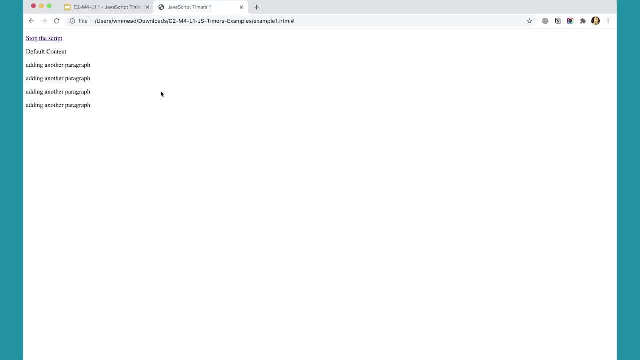 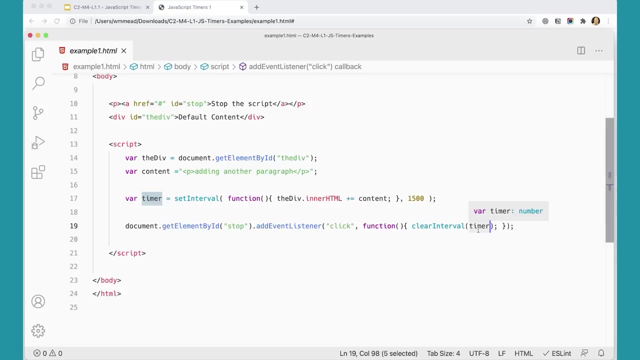 And when I click stop the script, then that event listener fires and it runs the clear interval. It runs a function with clear interval in it and then stops that script. It clears the interval timer. Now we don't need to do this. 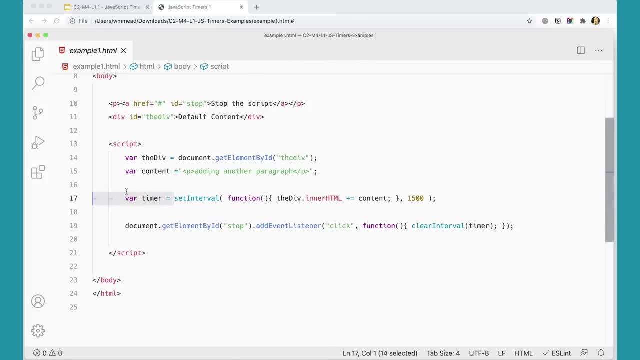 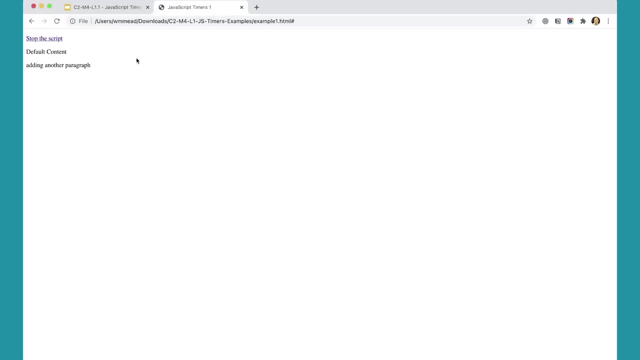 We don't need to use the function expression here. If I were to remove this, the page would still work, in that it would still run set interval and start adding div to the content. If I save that and come back here and refresh, you'll see it will continue to work. 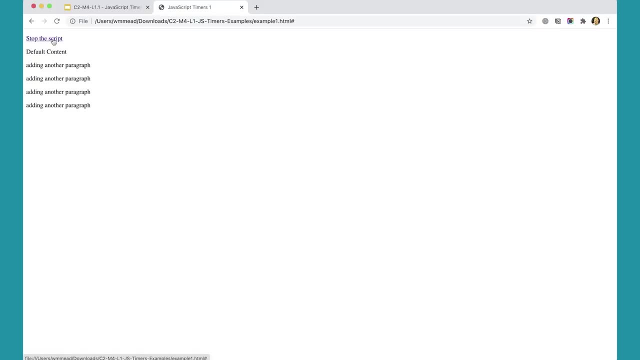 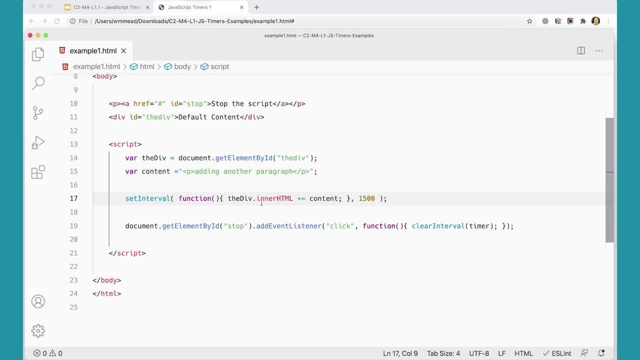 in terms of adding that in there. But the stop script function won't work. In order to stop the script I have to have this thing set to some sort of variable so that I can pass that variable into clear interval over here. The other option would be to just to put set interval inside there. 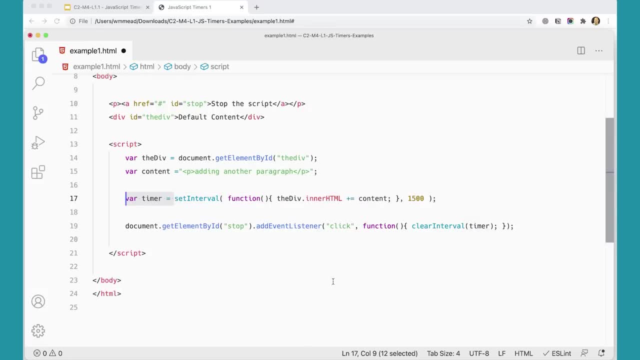 but then you need something to start it, to get it started. So, in order to clear the interval, I need to assign my set interval to a timer- It's really the bottom line here- in order to make that work. So I'm going to go ahead and do that. 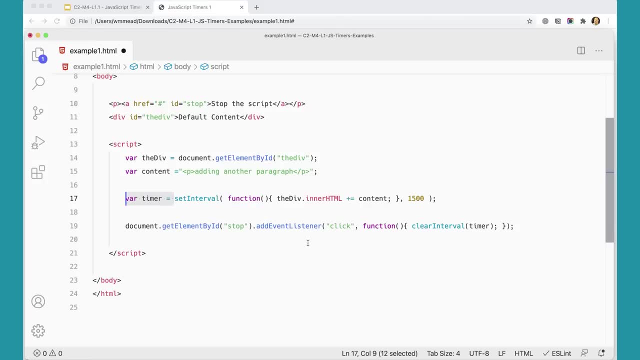 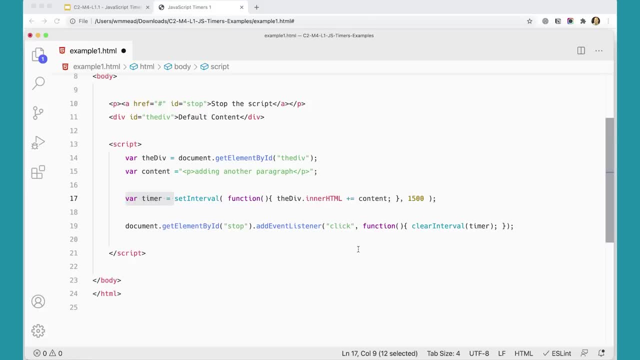 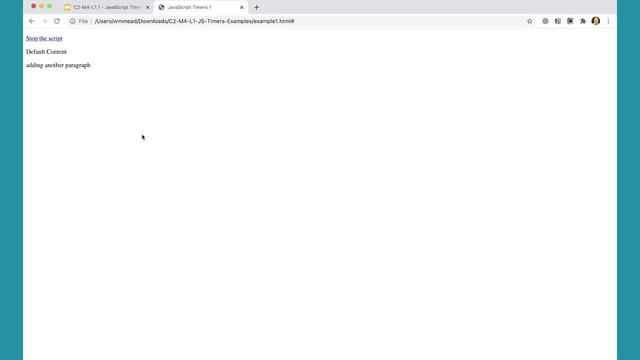 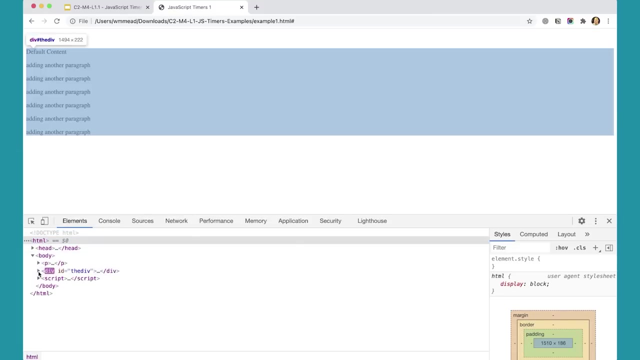 Now there's one other thing that I'd like to be clear about with this script before we finish. If I go back here and refresh the page and right-click and choose inspect, what I'd like you to really notice here is that notice all of these paragraphs are. 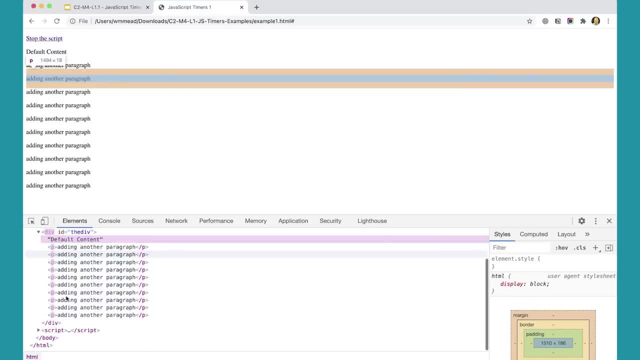 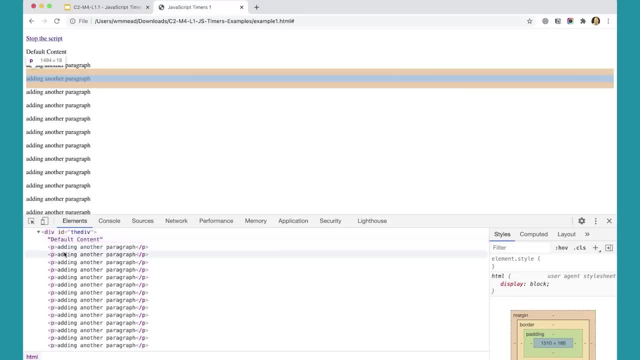 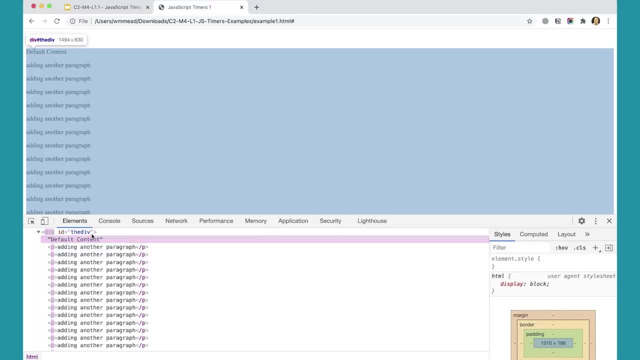 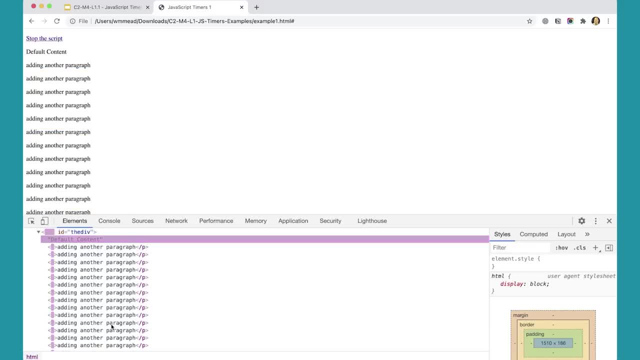 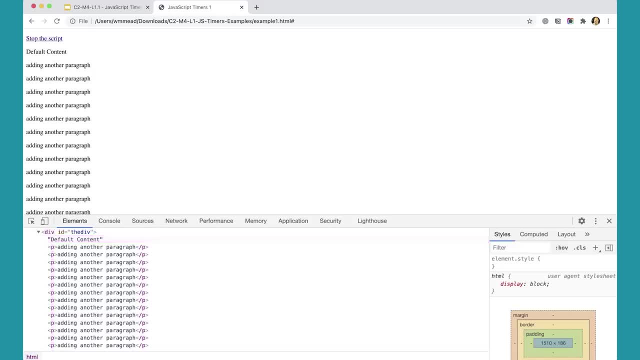 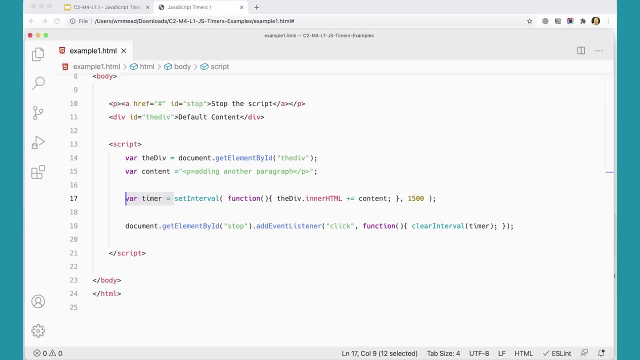 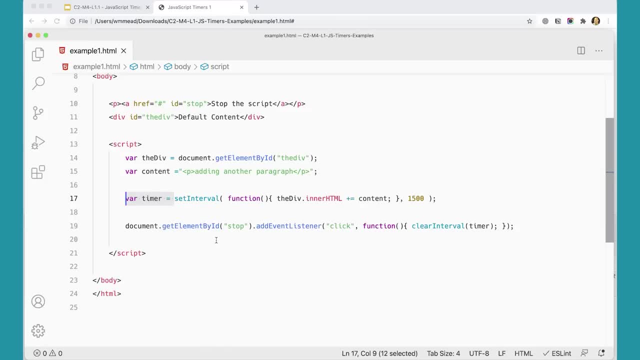 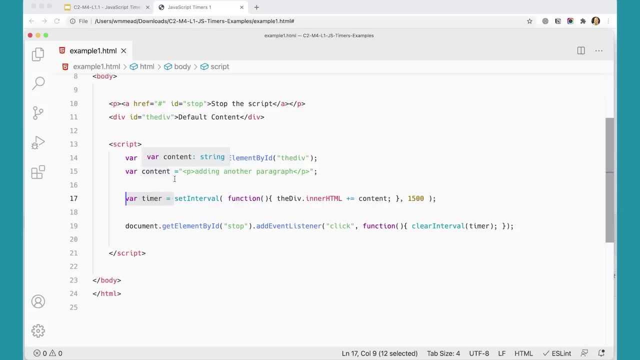 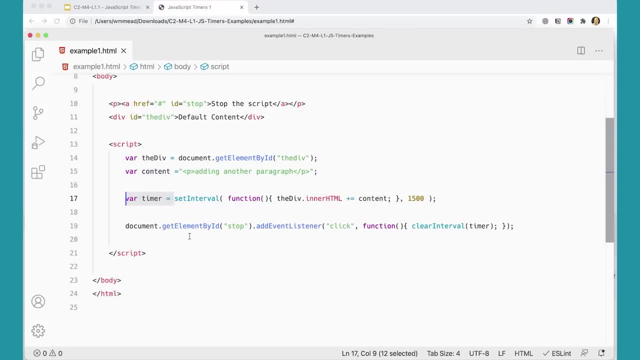 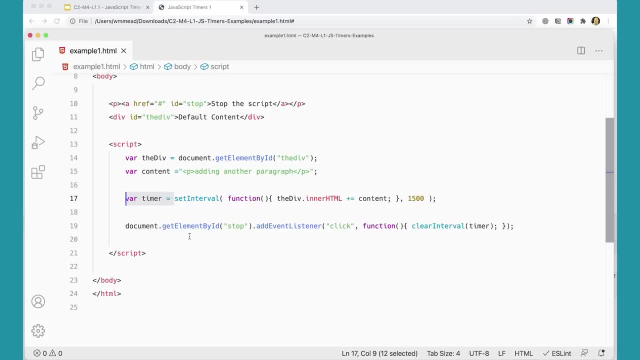 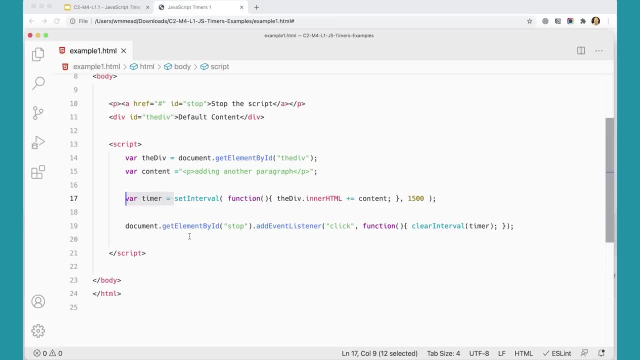 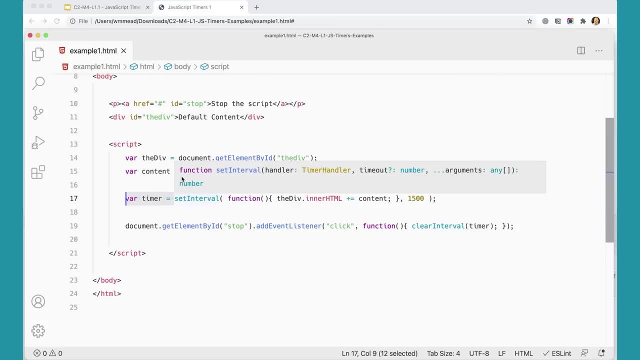 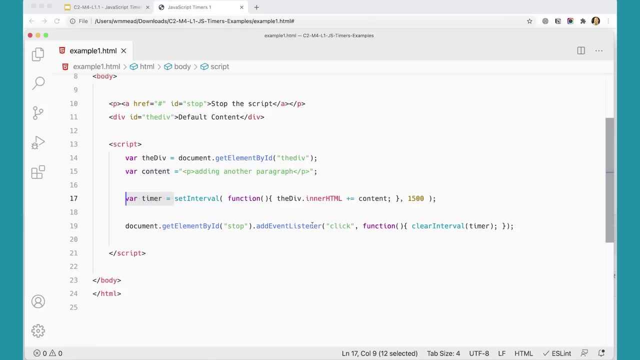 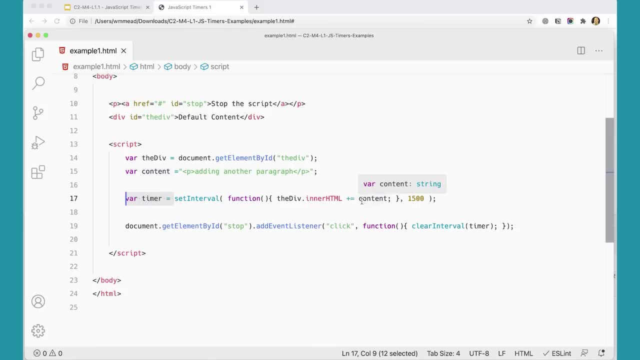 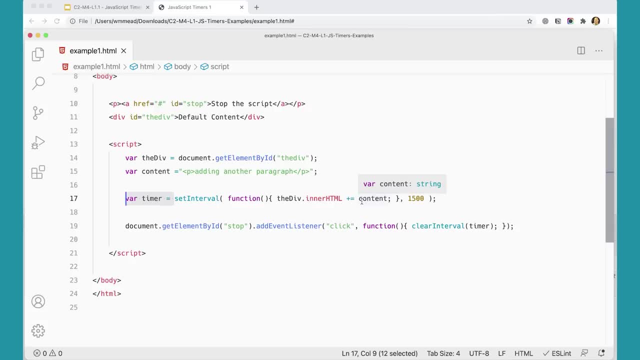 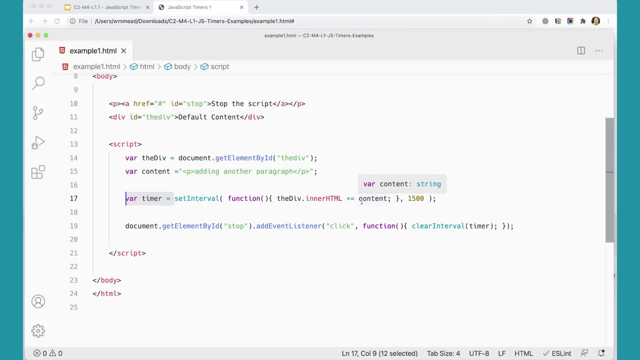 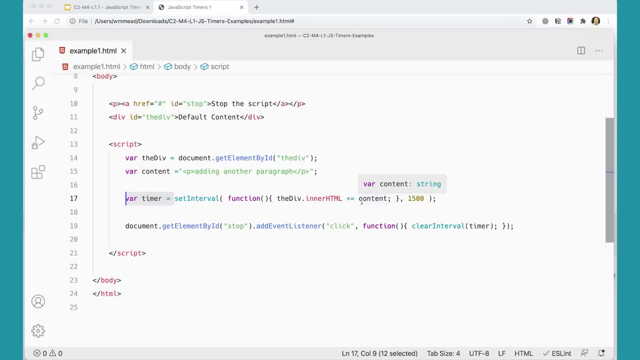 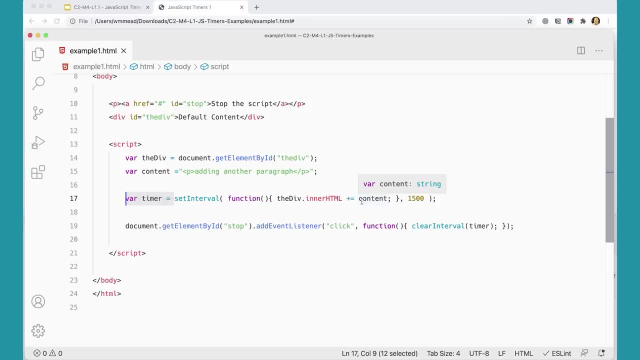 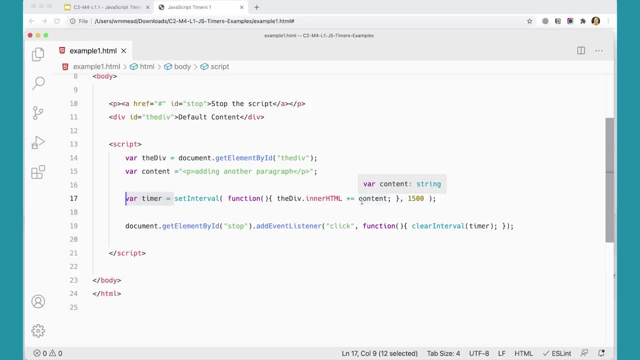 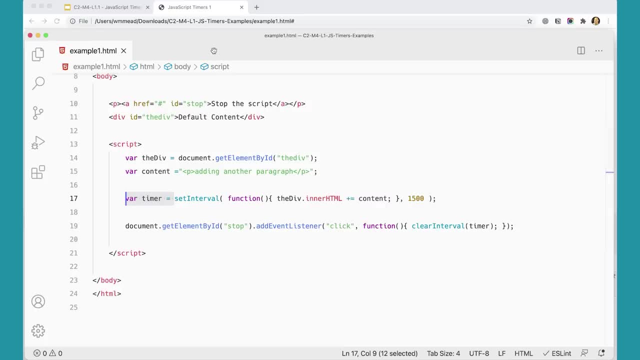 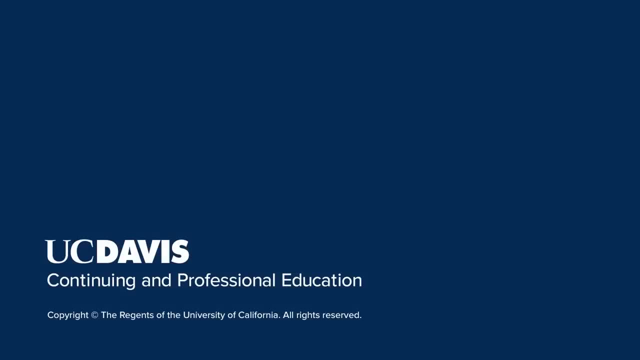 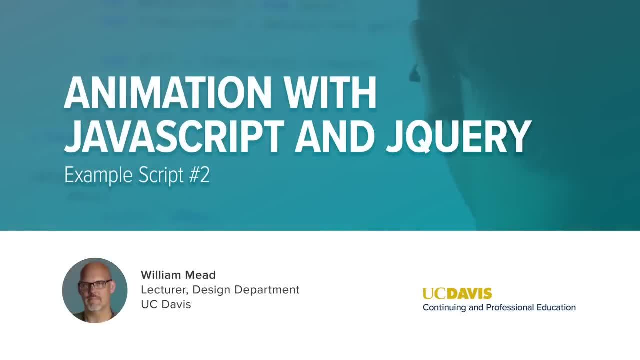 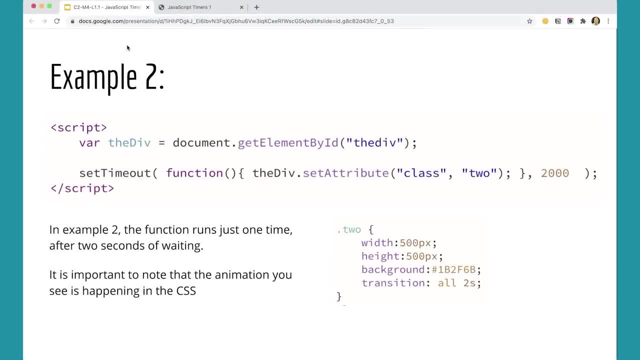 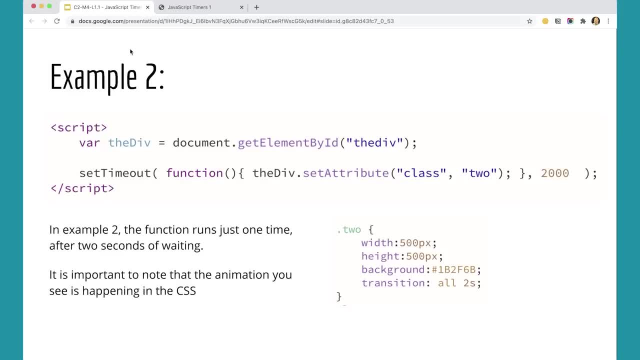 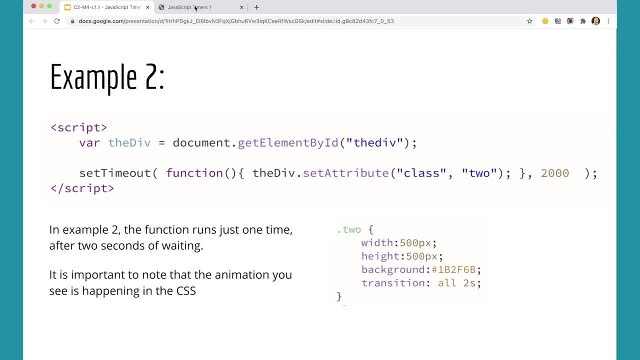 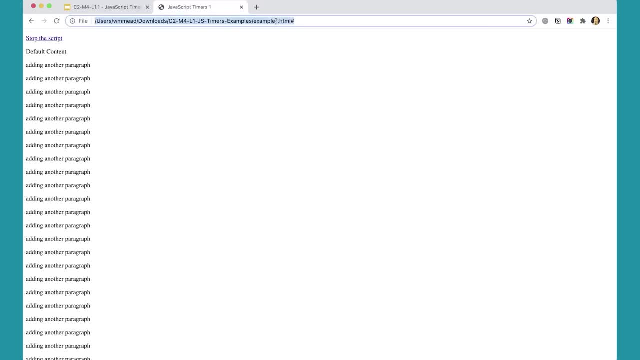 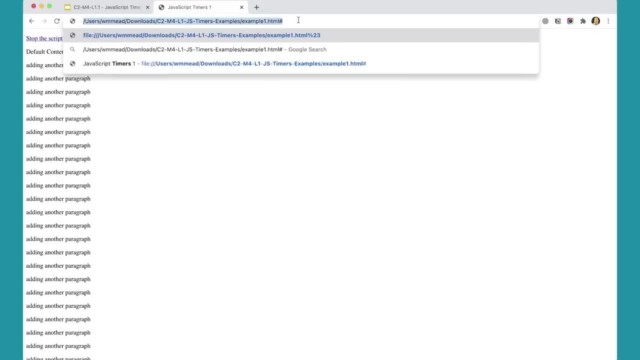 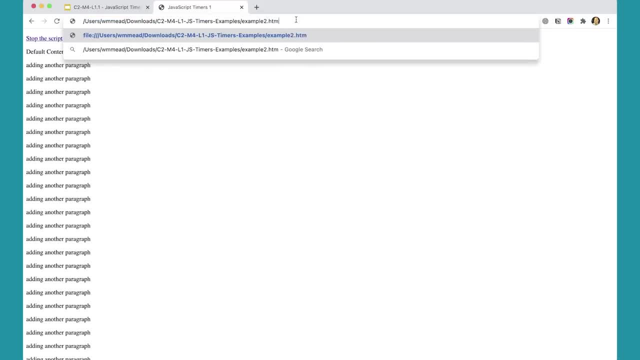 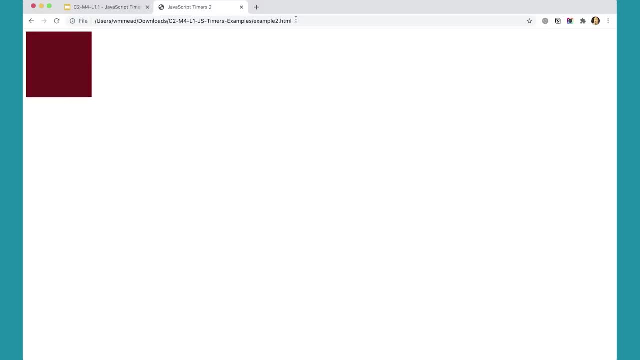 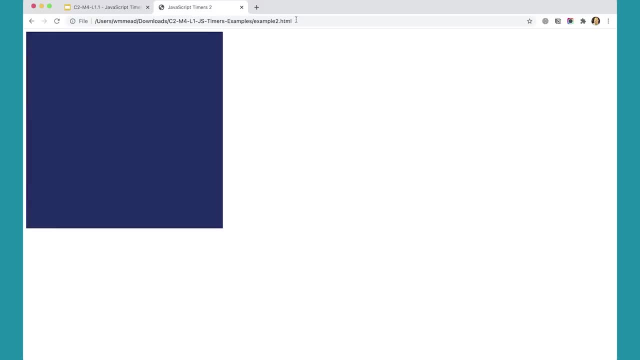 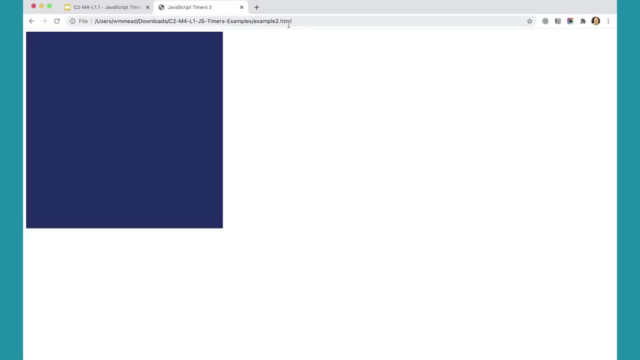 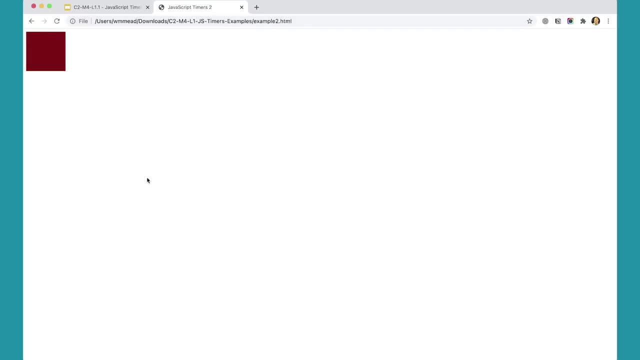 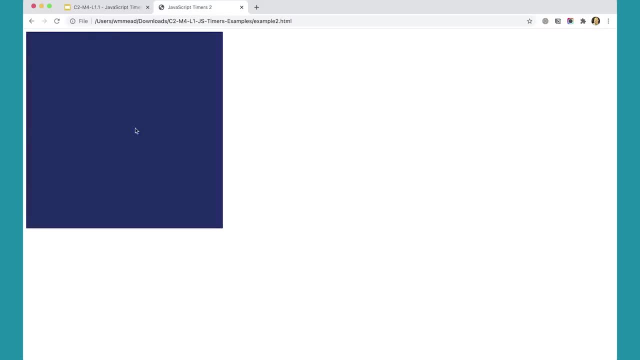 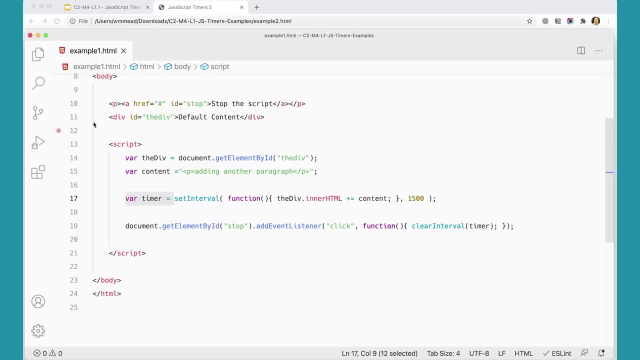 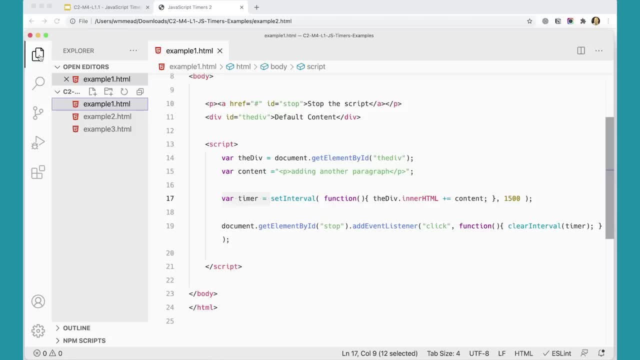 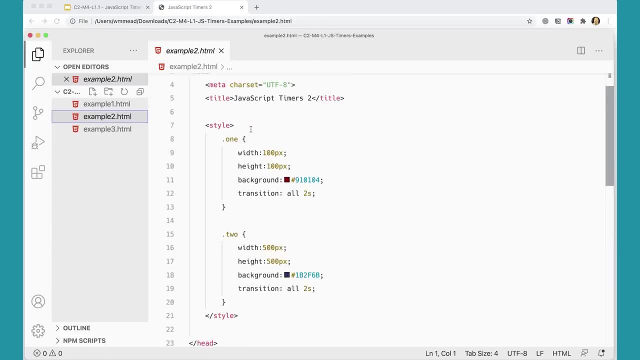 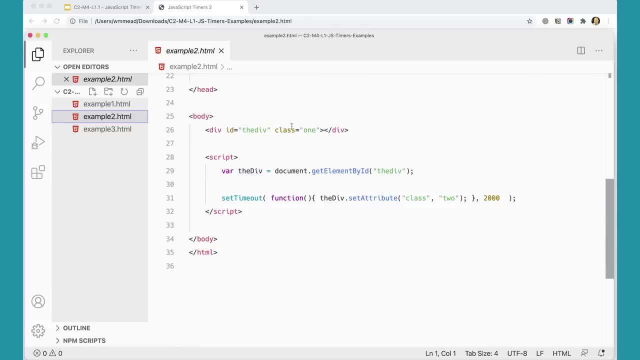 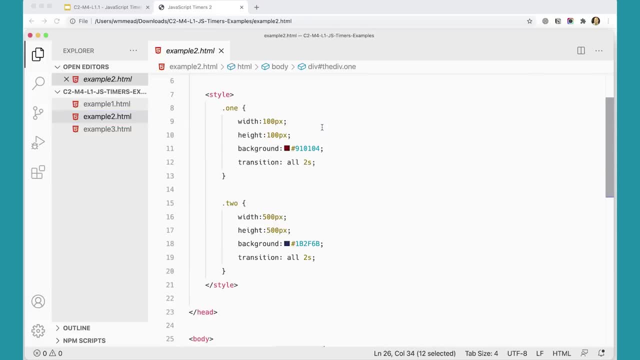 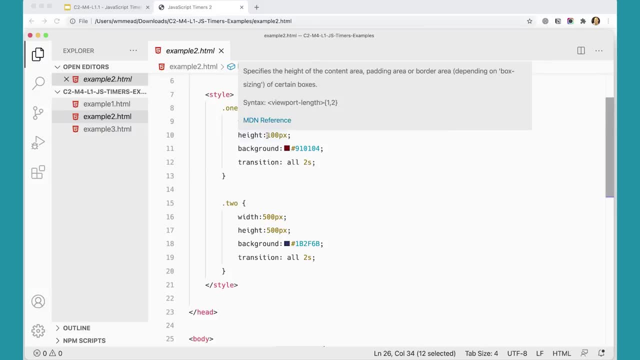 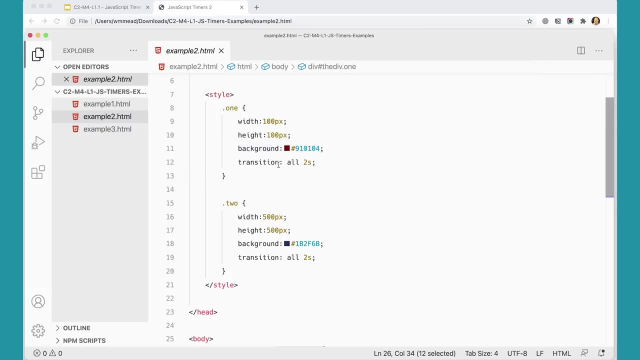 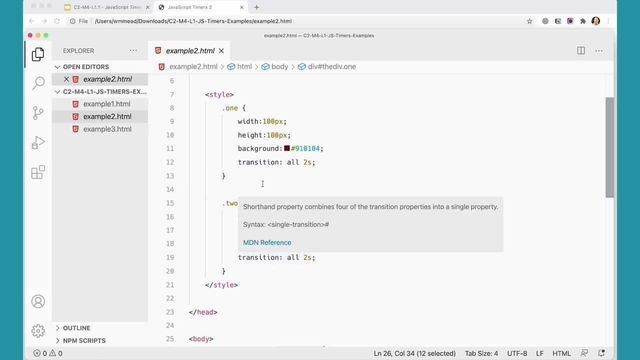 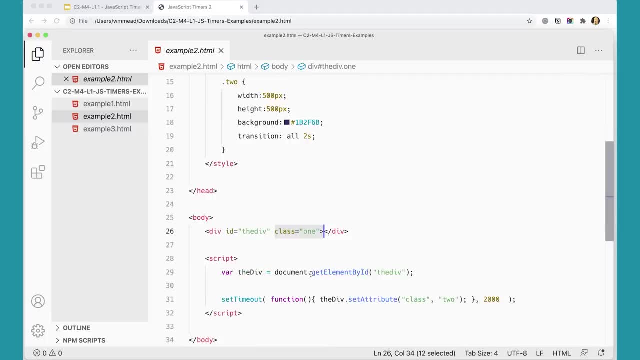 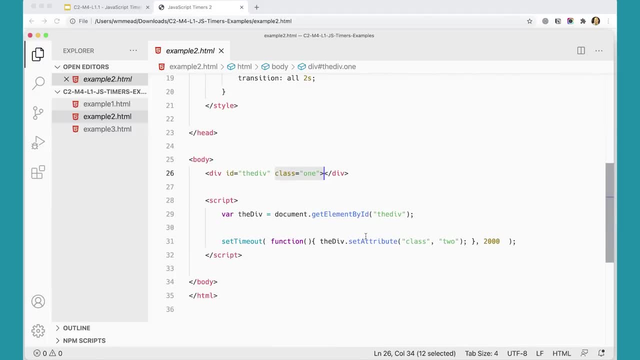 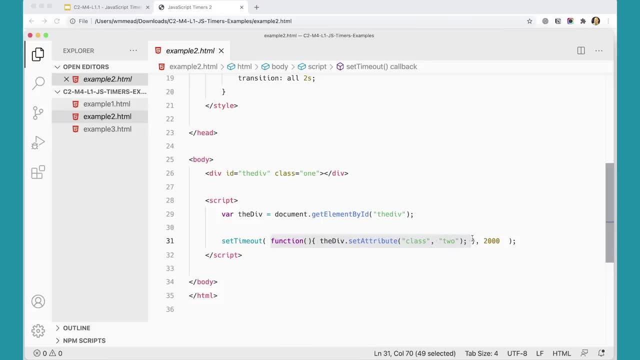 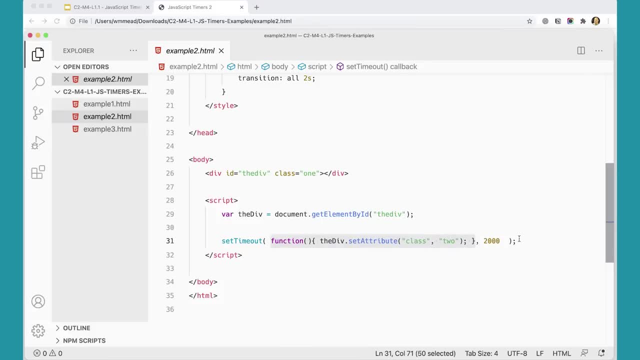 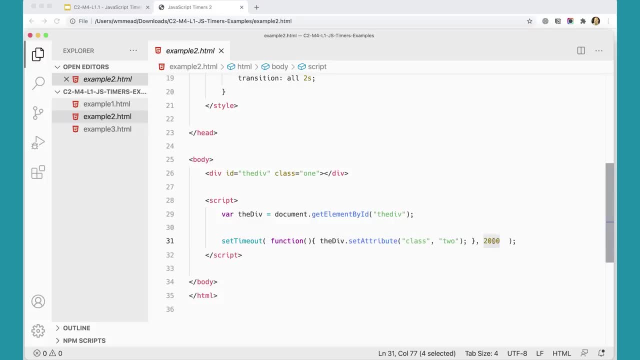 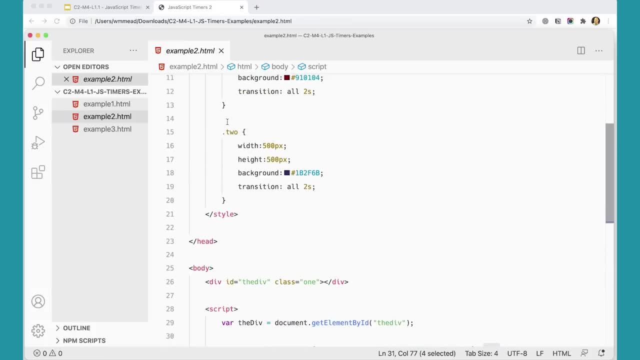 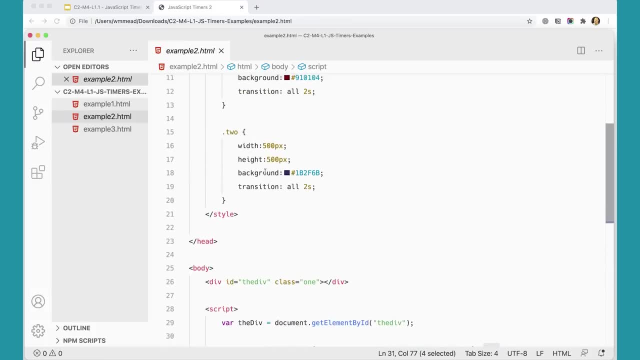 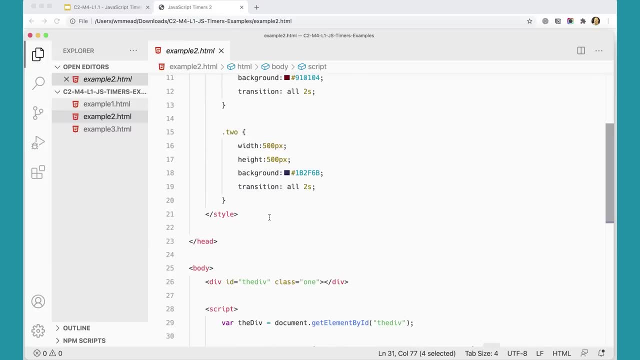 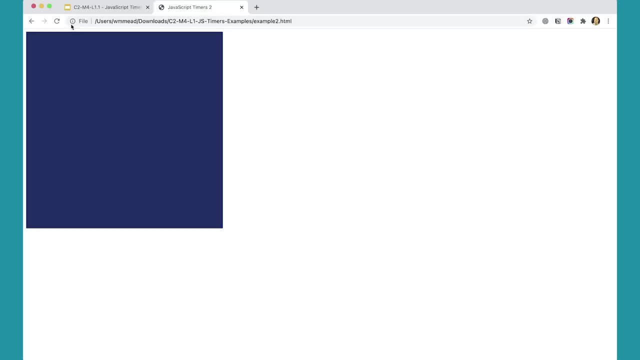 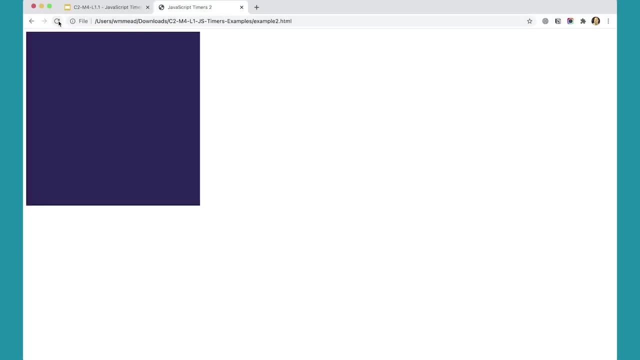 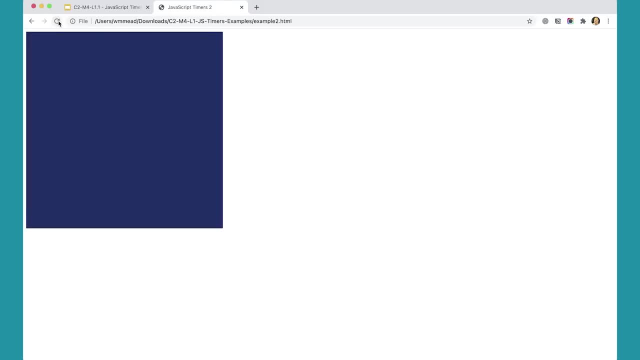 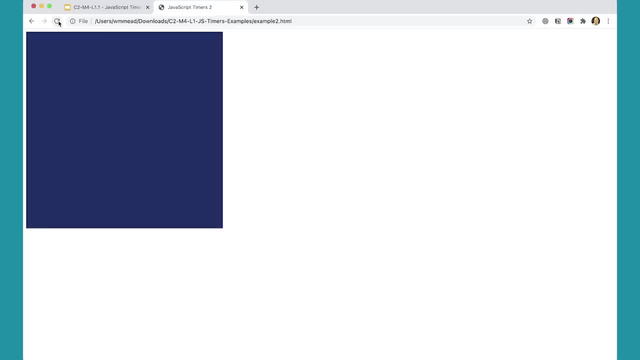 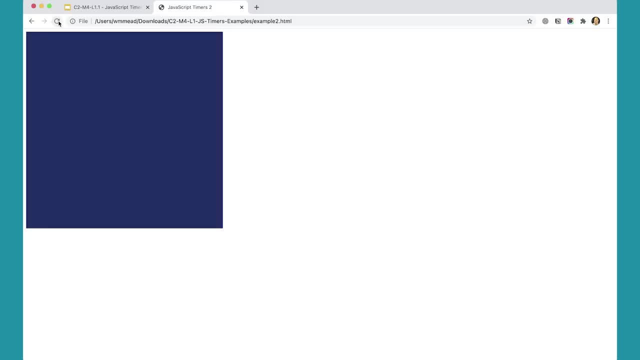 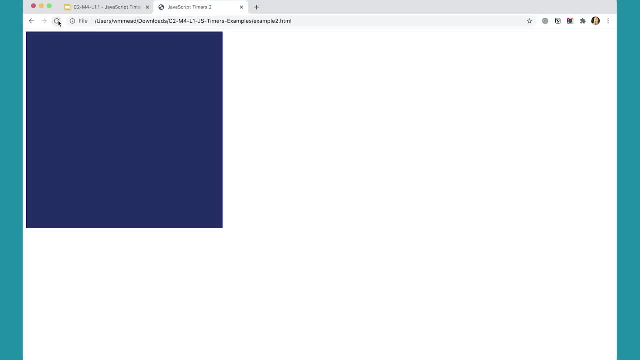 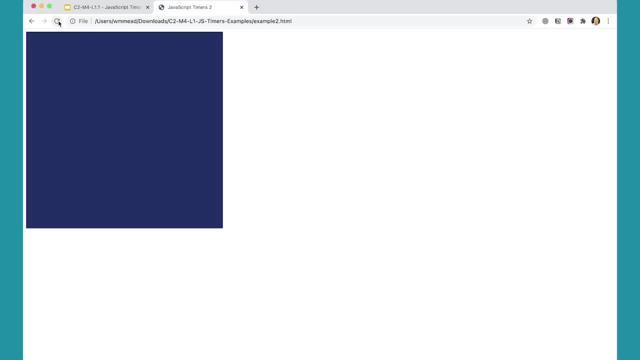 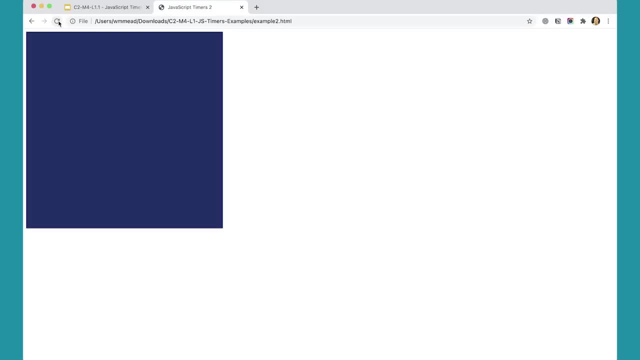 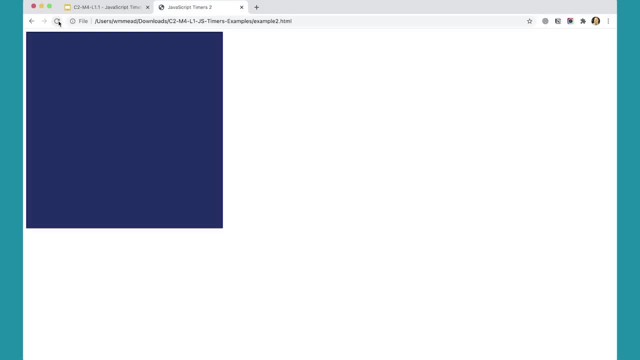 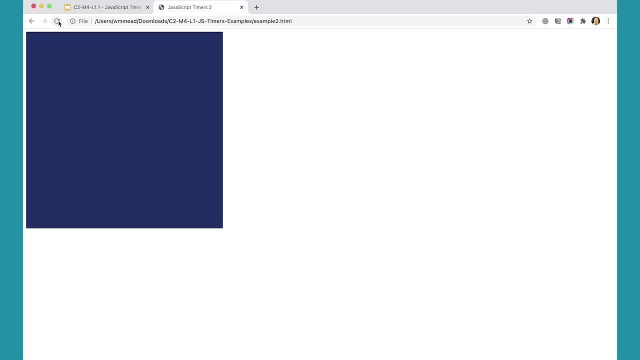 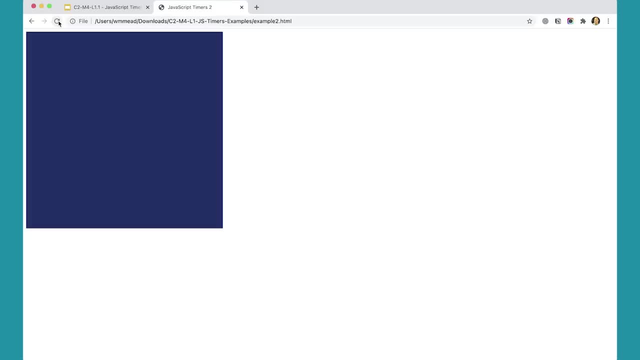 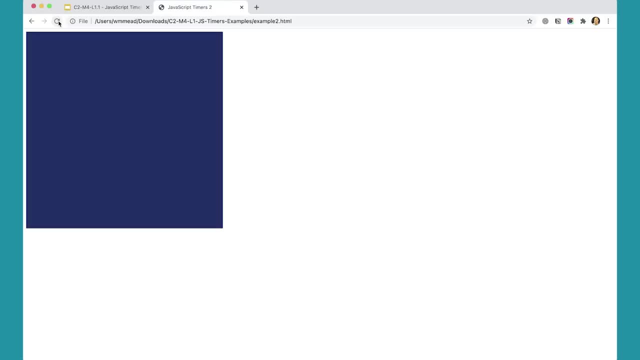 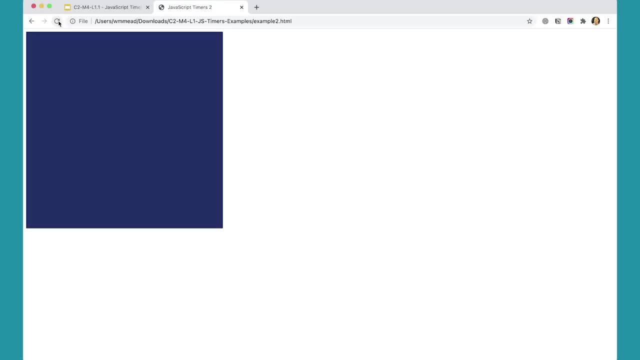 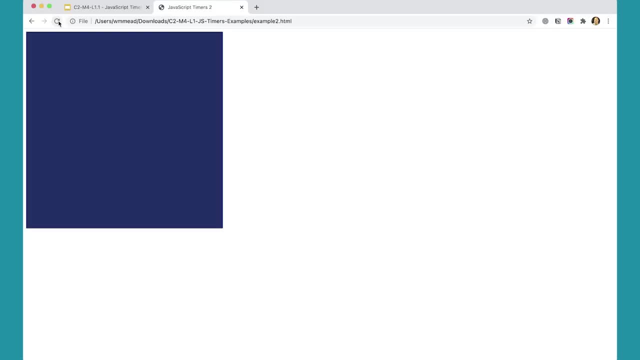 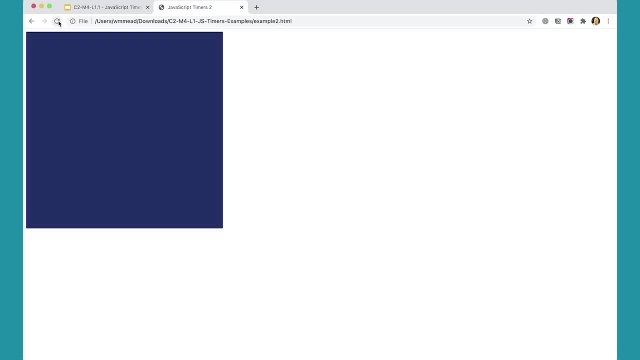 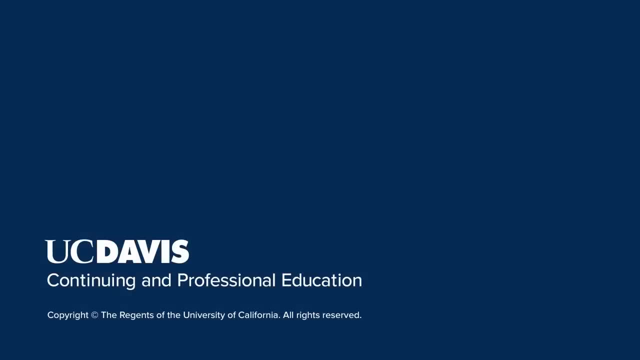 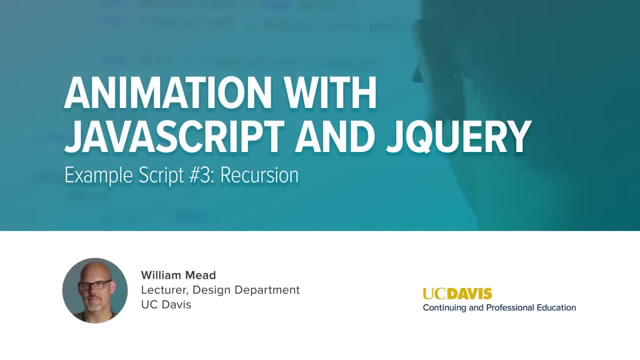 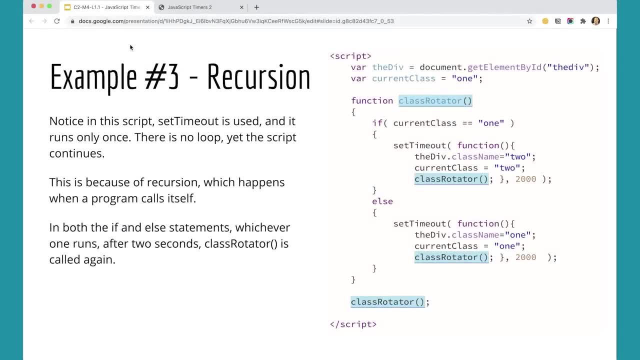 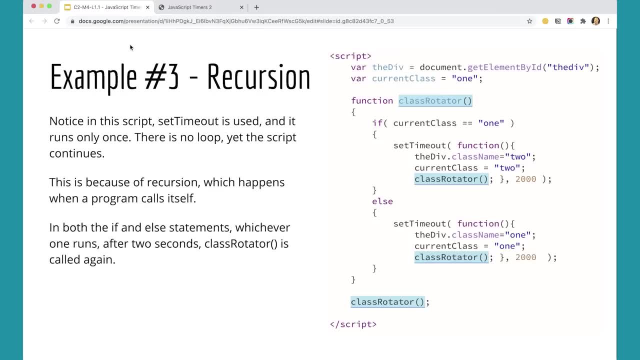 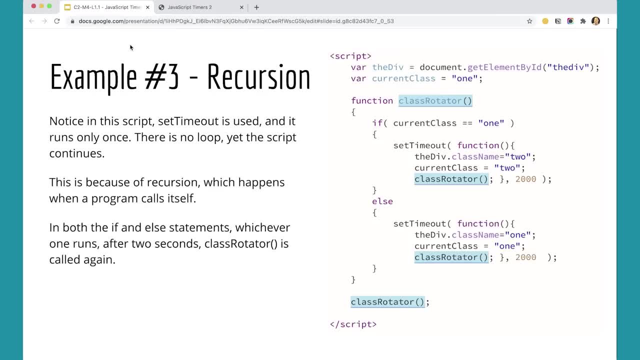 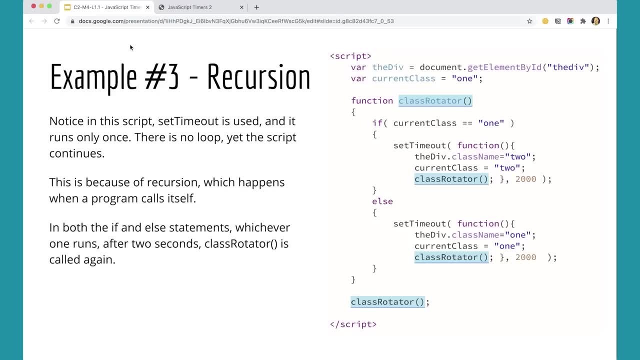 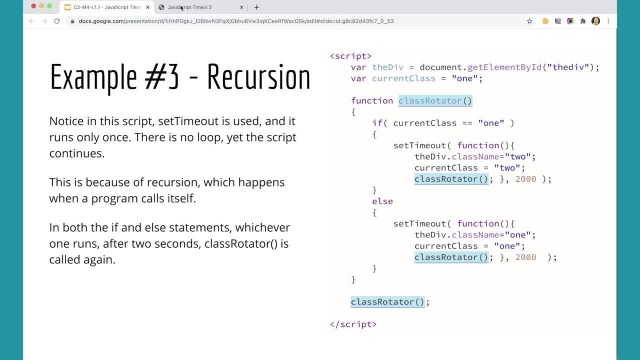 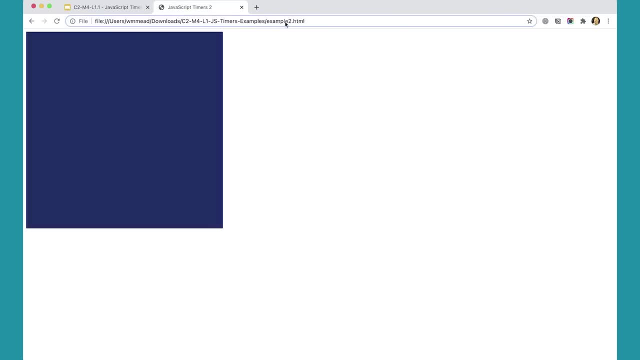 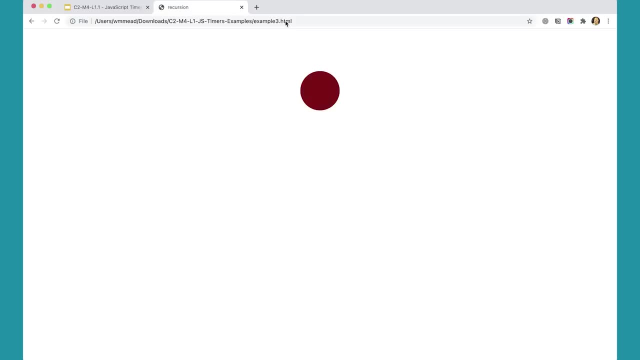 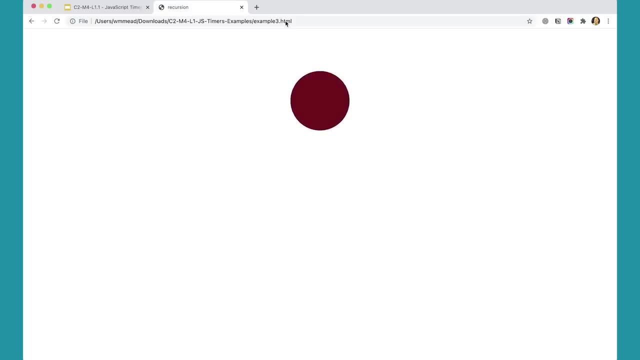 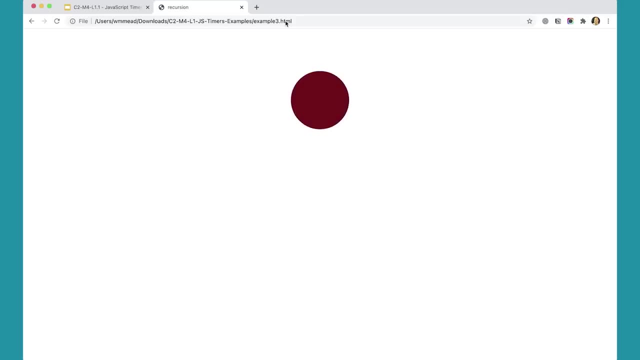 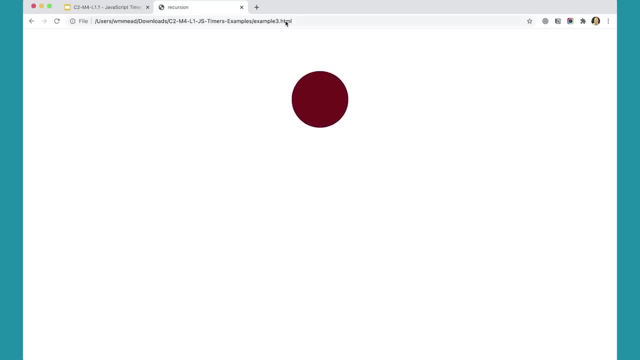 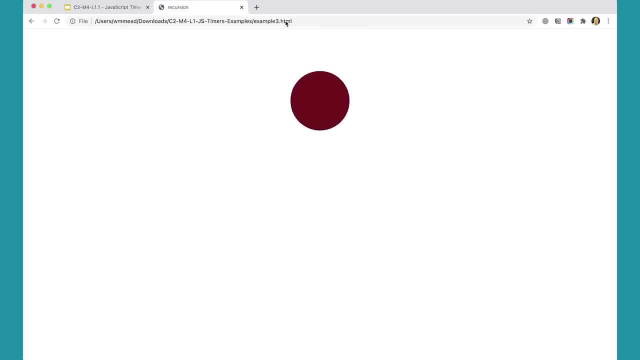 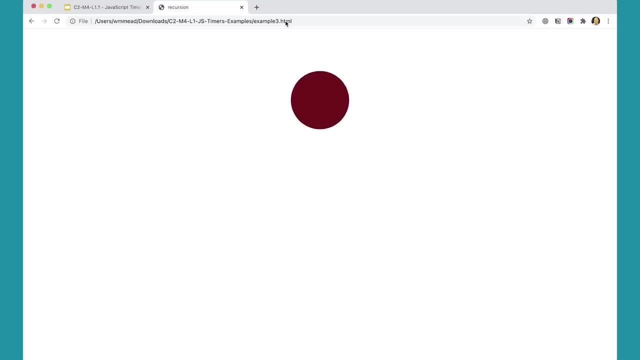 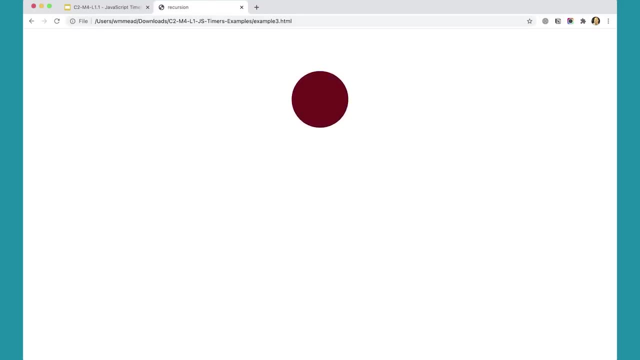 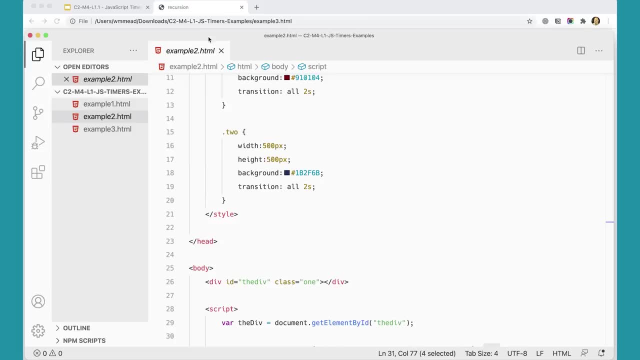 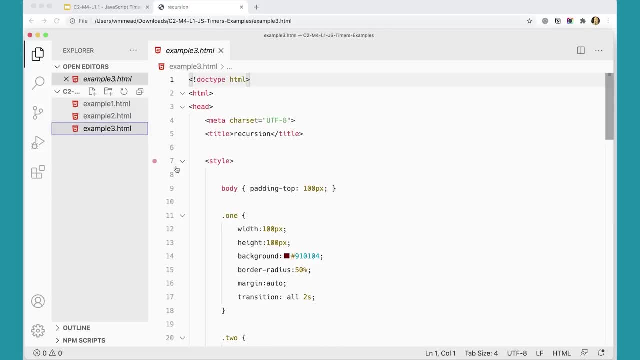 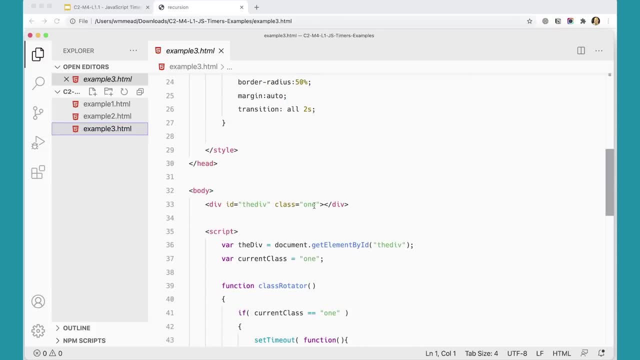 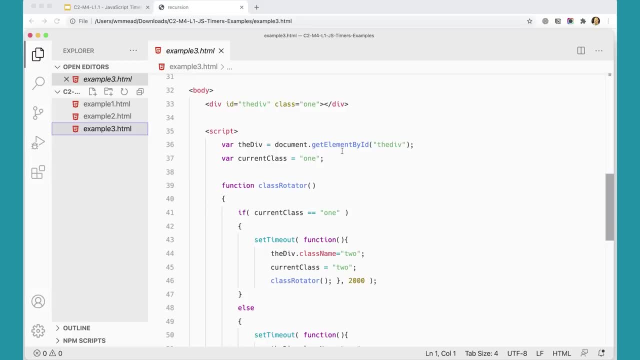 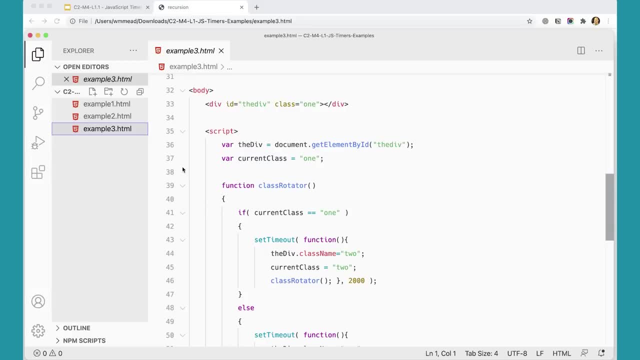 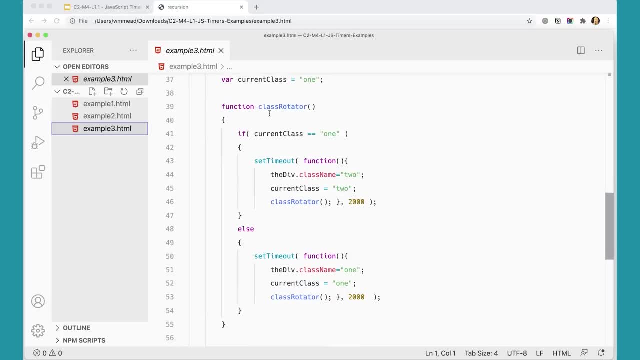 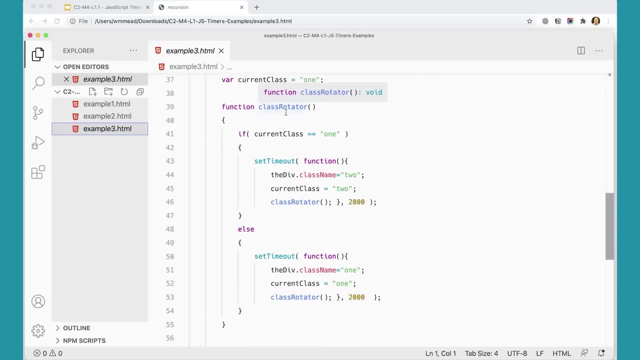 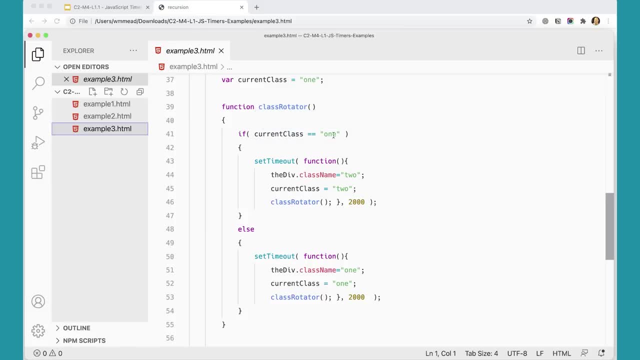 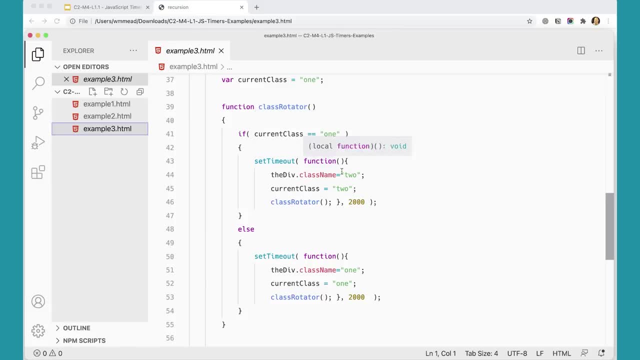 Notice all of these paragraphs are highlighting every time this script runs. Notice, all of these paragraphs are highlighting every time this script runs. and I'm going to run a function that's going to run after two seconds And in this function I'm going to take the div and set the class name to two. 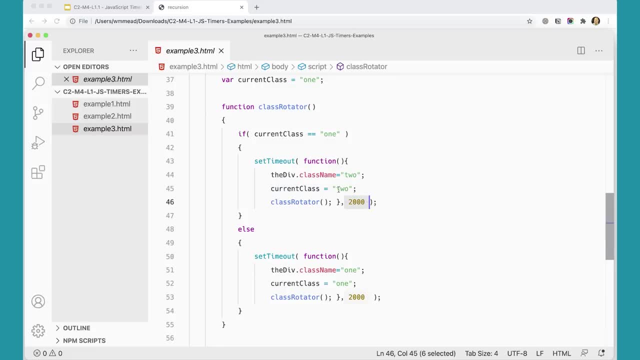 And then I'm going to set current class up here to two. So if it's set to one, set it to two. If it's not set to one, then it must be two, in which case I should set it to one and set current class to one. 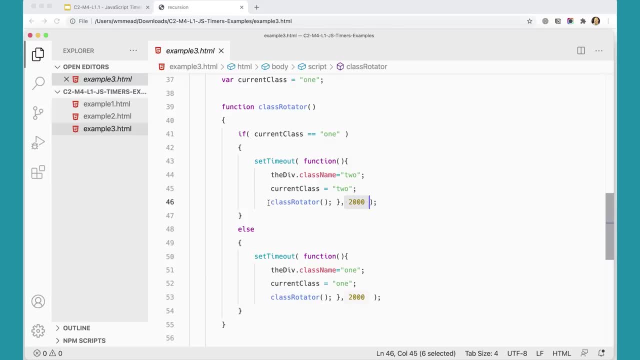 and run it over two seconds, But notice that this function is running class rotator. So a recursive function is a function that calls itself, And this is an example of a function that calls itself. It calls itself here and it calls itself here. 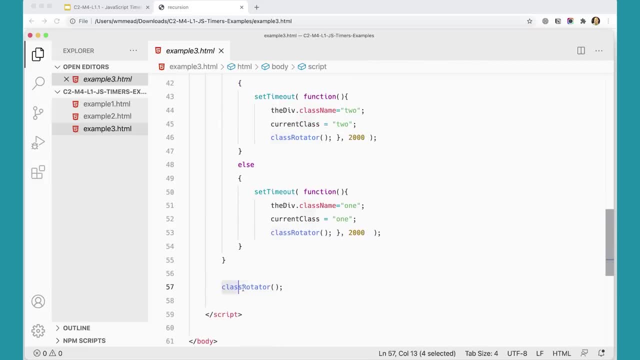 To kick off the function entirely, we have to run it once down here. So when the page loads it runs this once, But then when it runs itself, it either runs itself again here or it runs itself again, Depending on what's going on with the if statement and the set timeout. 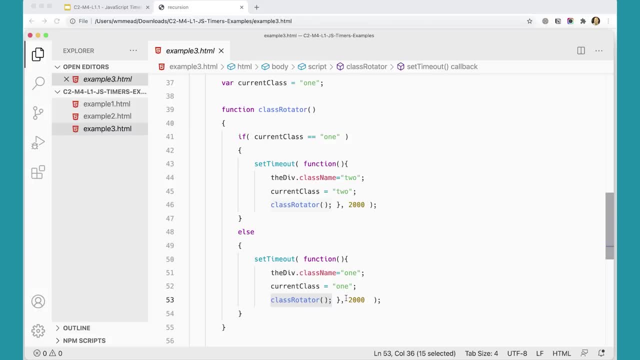 Now, recursion is a very powerful thing And it's easy with recursion to get confused or to do something that will cause your script to run out of memory and to run crazy and wild. So, for example, if I took class rotator here and just stuck it outside of the set timeout, 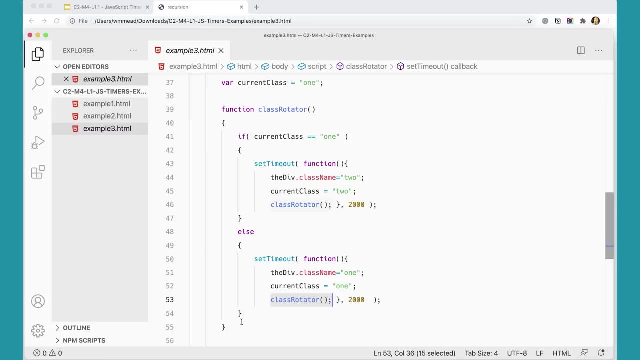 it would run very quickly and it would keep running itself and they would start to get stacked up and eventually you'd run out of memory. You'd get a heap overflow error showing that, basically, JavaScript has run out of memory, And that can happen very easily. 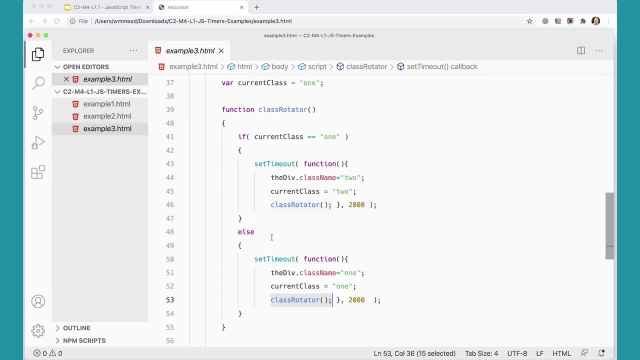 when you're working with recursive scripts. But when handled properly, recursion can be a very powerful feature, And not only that: it can be the preferred way of actually working with data and working with set timeout or set interval If, for example, you're going out to the world. 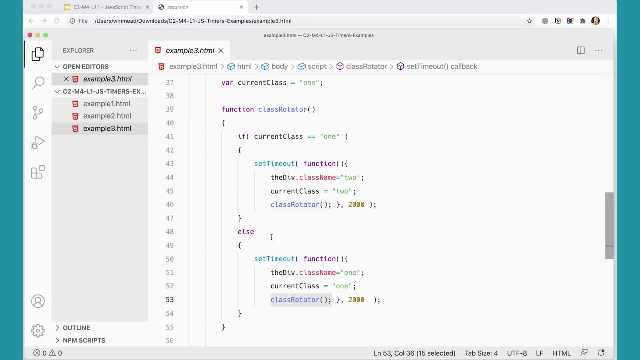 and getting a piece of data from somewhere and then doing something when it comes back. usually, recursion is the better way to go, because you can wait until it's come back before you try to do something with it, Whereas if you use set interval, then you're more likely to try to do something. 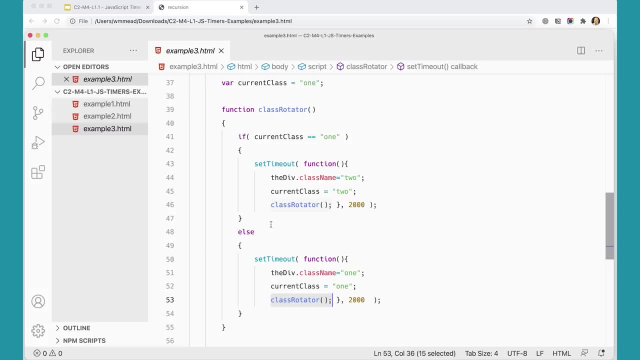 before you get your data back. Set interval will run every X amount of seconds. Set timeout will wait at least two seconds, but maybe longer depending on where something is in the stack of things to run with JavaScript, And we'll get more into the event loop in JavaScript. 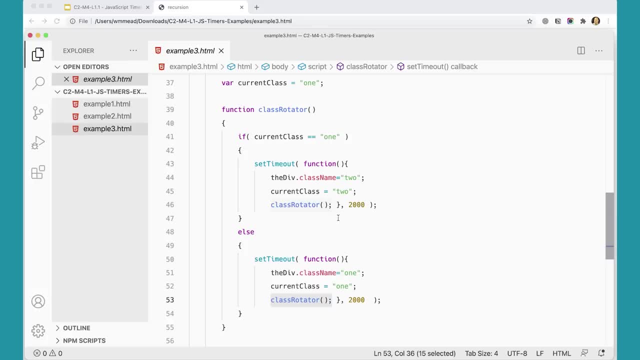 and talk more about how that works and why it is like that in a later lesson, But for right now, I just want you to bask in the glory of looking at what happens with this, because I think it's really kind of interesting. 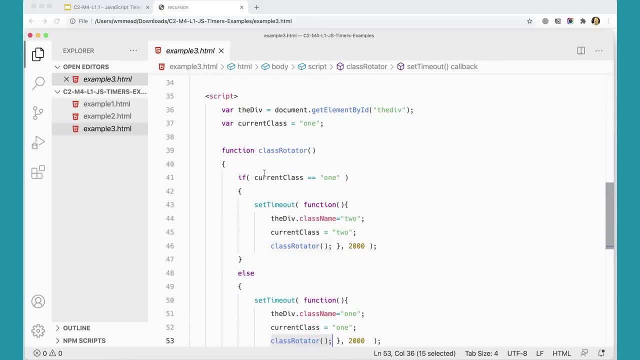 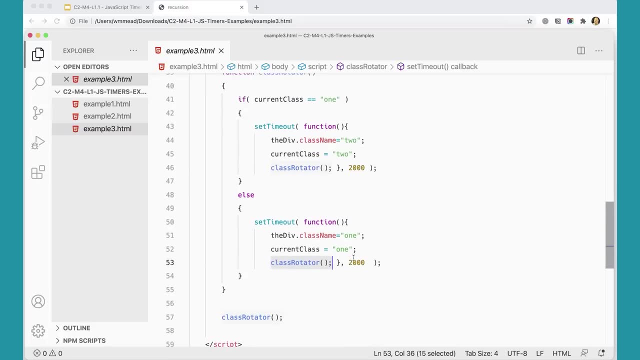 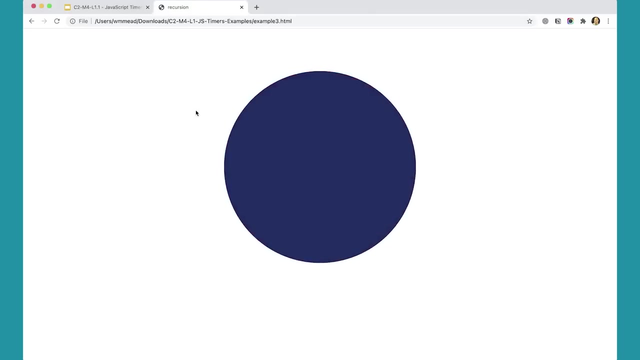 I've got two classes and this function is calling itself, but it's only calling itself after two seconds has lapsed, either here or here, And that gives us this very interesting, very interesting pulsating kind of creepy circle that feels like it's breathing on our web page. 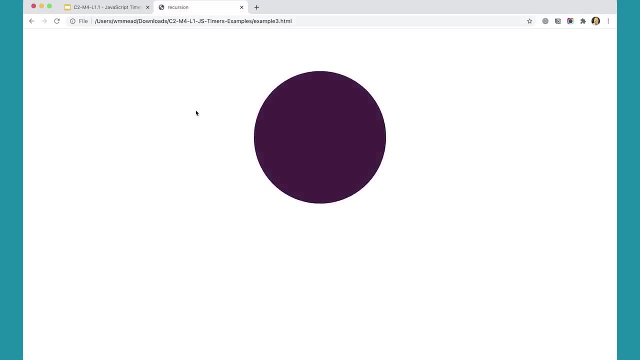 And you could do. you know more stuff for that if you wanted to. Okay, So with these techniques we can do a lot of really interesting things. You could do interesting things with games. You could do interesting things with other types of scripts. 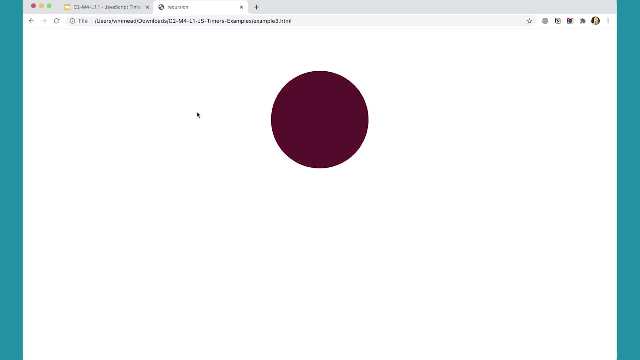 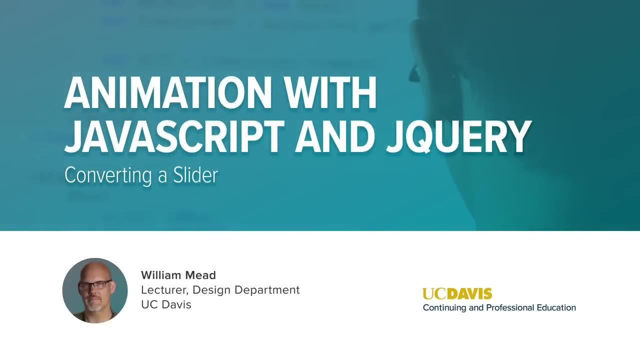 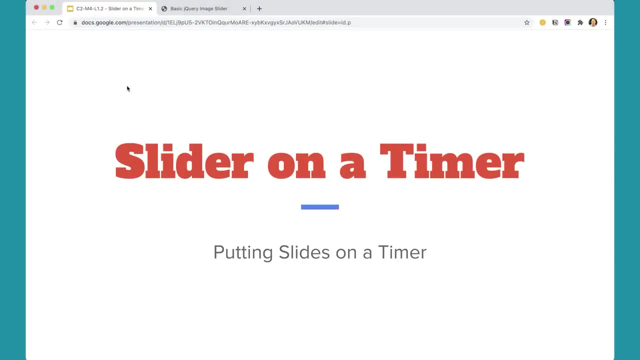 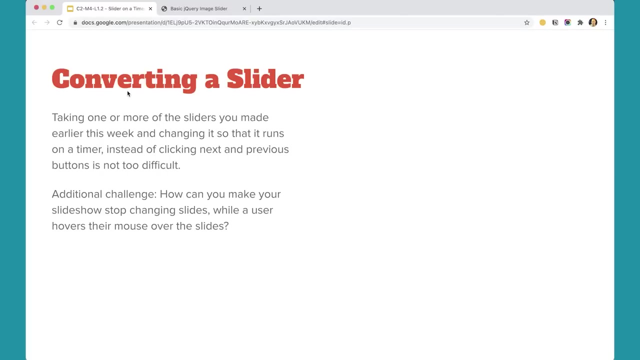 where you want them to run automatically on some sort of timer. Sliders on a timer. Sliders on a timer: Putting slides on a timer. In this lesson we'll convert one of the slideshows that we did in the previous module to. 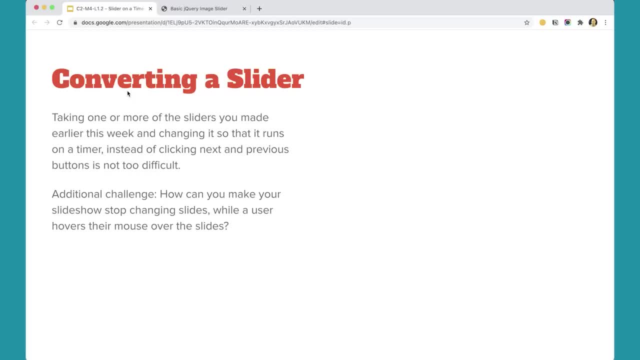 so that it runs on a timer without having to click the next and previous buttons, so that it runs automatically And you could pick any of the three that we did in the previous lesson, or if you figured out how to take the JavaScript-only one and make it run on a never-ending loop. 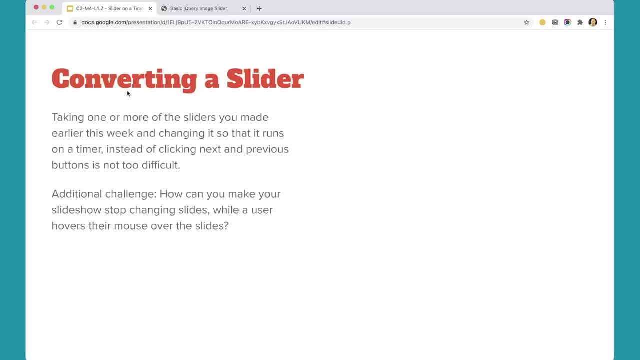 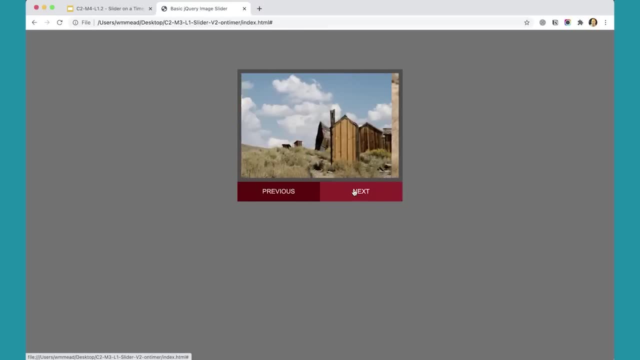 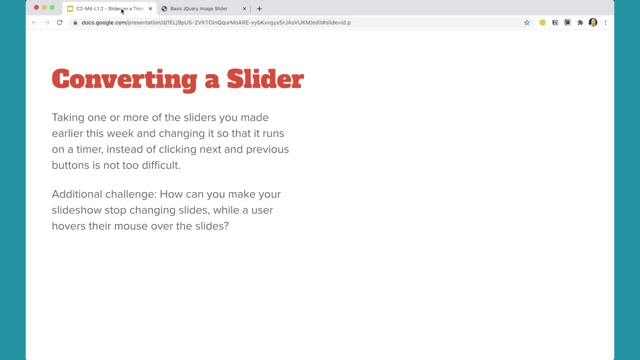 you could use that one. You could use any of them. So I'm gonna use the slides here, this slider here that loops around and goes in any direction this way. Okay, going to make this one run on a timer Now, before you follow my lesson and follow these videos. 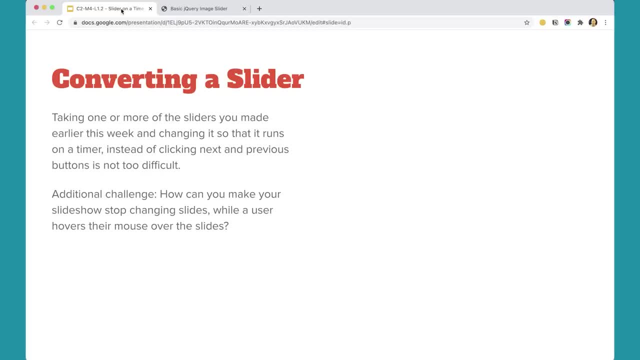 showing you how to do it. I strongly encourage you to try to do it for yourself- It's not that hard- and see if you can actually figure it out. See if you can get one of your sliders to work on a timer To do that. get rid of the buttons. Delete the buttons off the screen. You can delete the CSS. 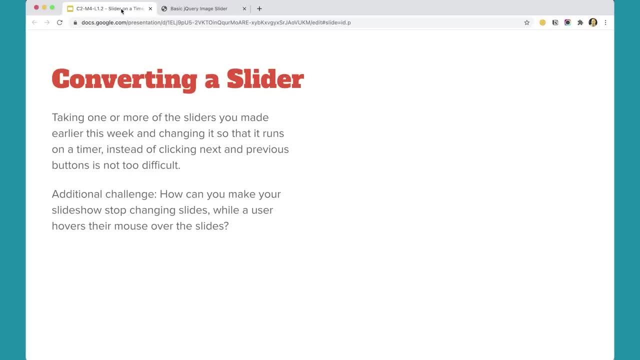 that has to do with the buttons off the files, and then modify the script so that it's using setInterval or setTimeout, using recursion, Either one of them. You can make it work either way. So use one of those two methods and see if you can create your slider so that it works. 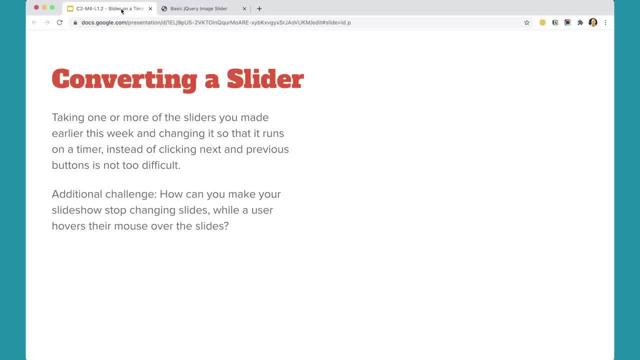 As an added challenge, make it so that when the user hovers their mouse over the slides, the slides will move. When the slider stops, it stops doing its automatic moving forward of the slides And then when they move their mouse off of it, it starts again. That's kind of a fun challenge. 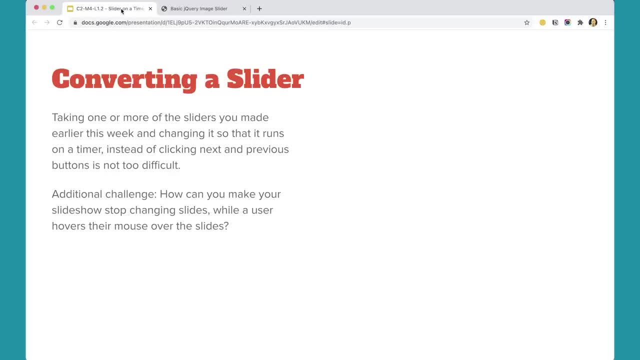 And it also happens to be a fairly useful interface technique, because if you have a slider on a web page, it's very possible that if you've got content or things in those slides that you want people to look at or read or do something with, it's kind of annoying when the slide 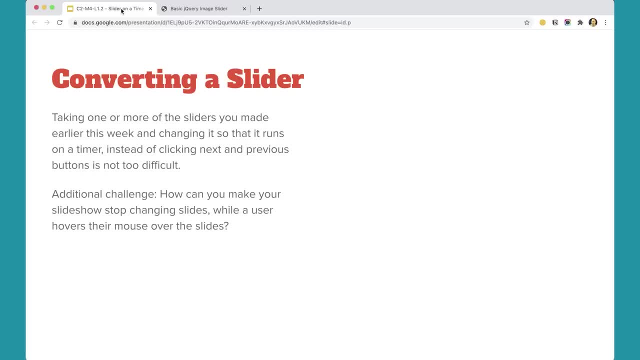 just automatically changes before you're done. So it's kind of nice if, while your mouse is hovering over that element, that it pauses the slider And then, when you roll your mouse off, the timer can kick back in and it will continue with the slides. Okay, so see if you can do that on your own And if 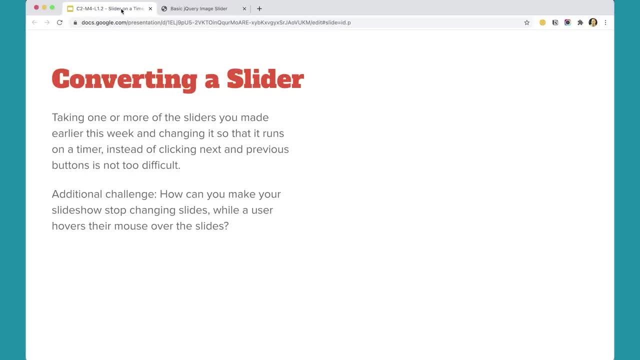 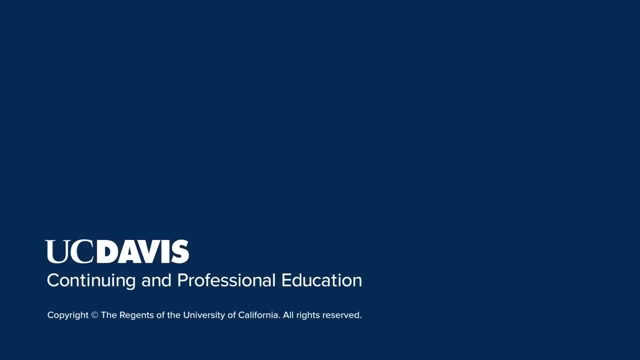 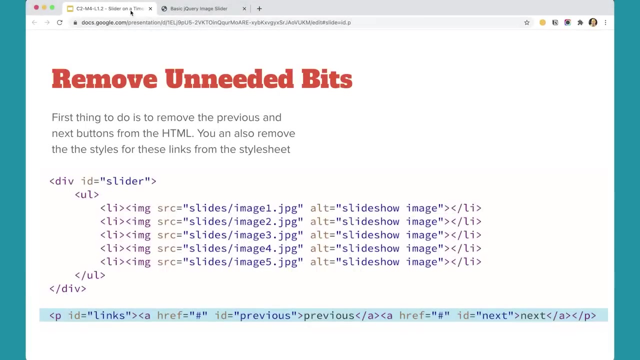 you get stuck or you want to see my solution? continue on with this presentation and with these videos. Hopefully, you were successful at creating your slider on a timer and were able to do that on your own, But if you weren't, or if you want to see how I did it, this is how I'm going to do it. 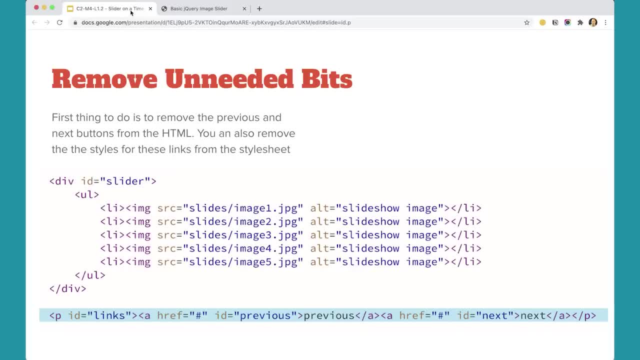 here I'll show you how I did it here. So, to start with, I'm going to go into my files and I'm going to remove this paragraph at the bottom that has the link has the previous slide. And I'm going to go into my files and I'm going to remove this paragraph at the bottom that has the link. has the. 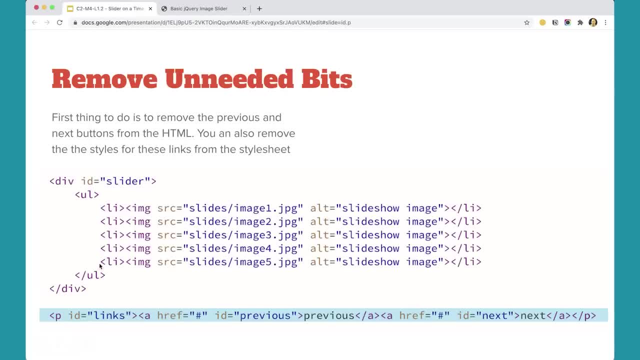 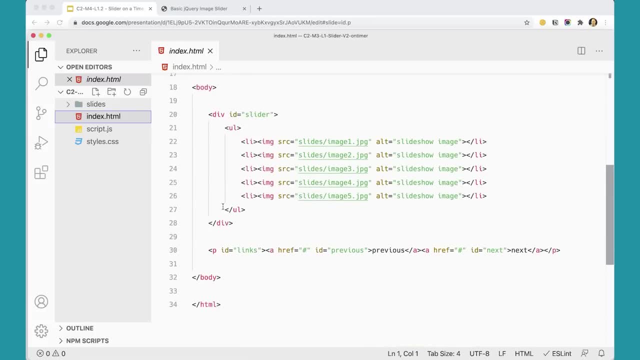 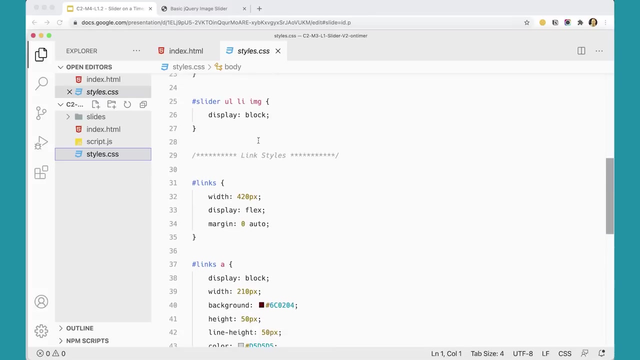 previous and next buttons because we don't really need those anymore. So I'm just going to come in here to my files here and go down and remove that there. Also, I might as well go over to my styles and remove the things that have to do with the styles that have to do the links. 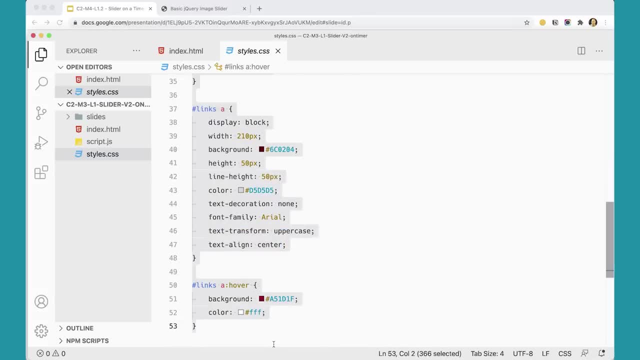 because I'm not going to use them anymore. I just think it's a good idea to remove unnecessary code if you're not using it. You don't really have to. It's not going to hurt anything if you leave it there. I just think it's a good idea. So now our slides will not have. 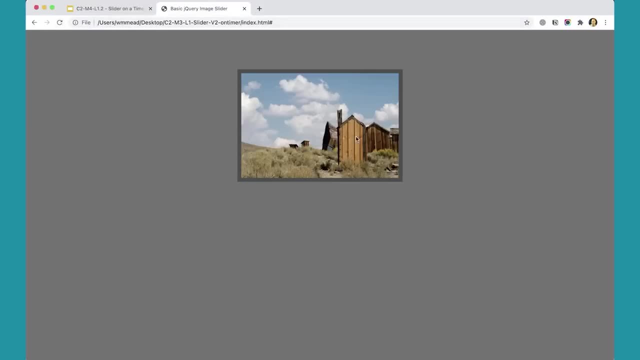 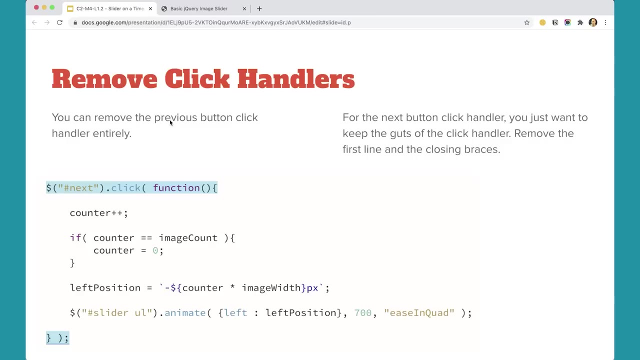 buttons attached to them. It's just going to be an empty slider, So we don't have a thing that we can click on. So the next thing we need to do is remove the click handlers. For the next click handler, I'm just going to remove the first line here. 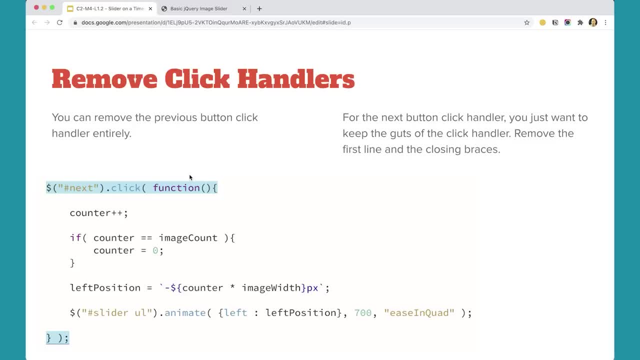 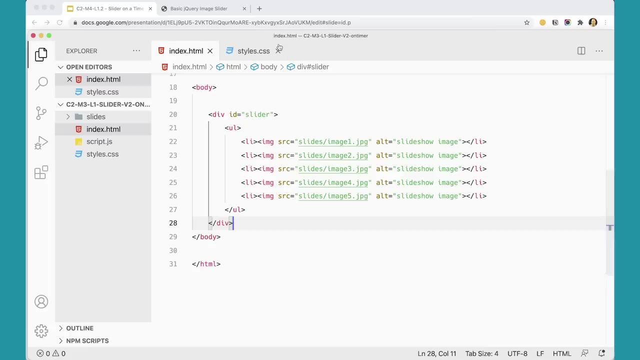 And the last line of the click handler and leave the guts For the previous click handler. we can just remove it entirely. So let's go over here and do that. next, Done with styles, Done with this file, We can go into our script. 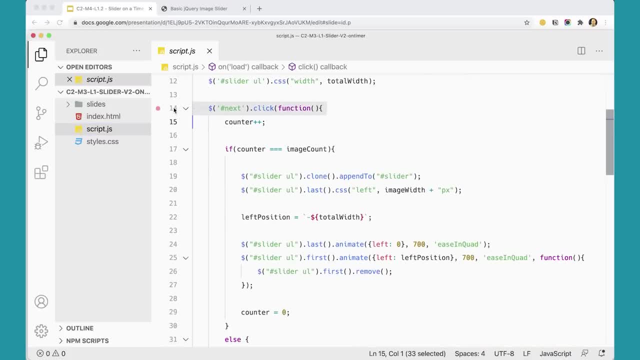 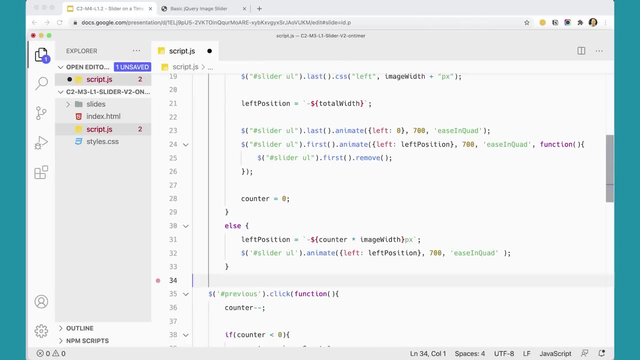 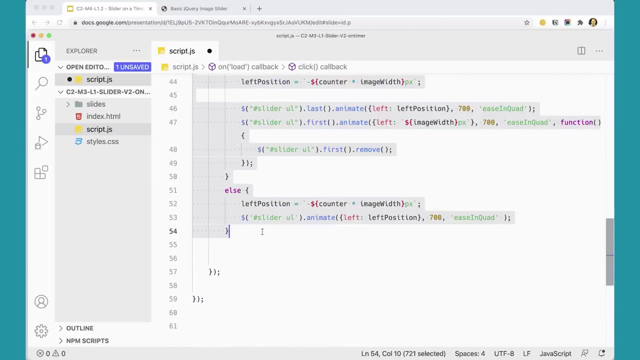 And I'm going to remove this line for my next click handler And the closing one down here, And then I don't need the previous one at all, So I can just get rid of all of this down to here- Actually, down to that one there, I think, Yep. 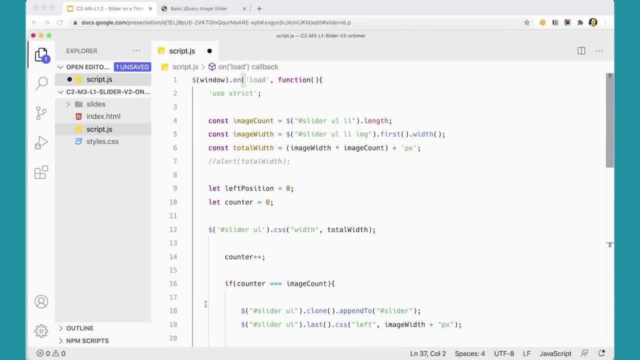 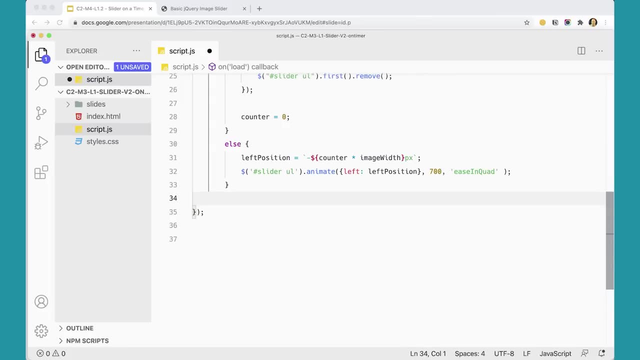 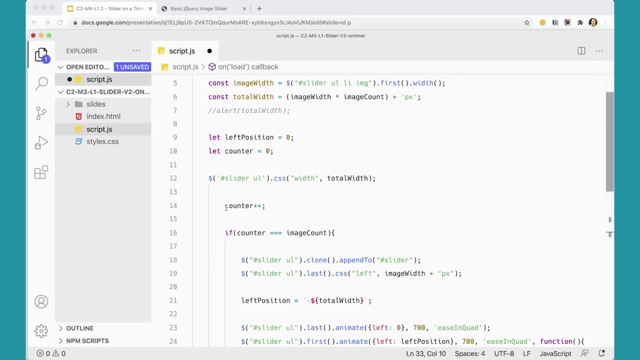 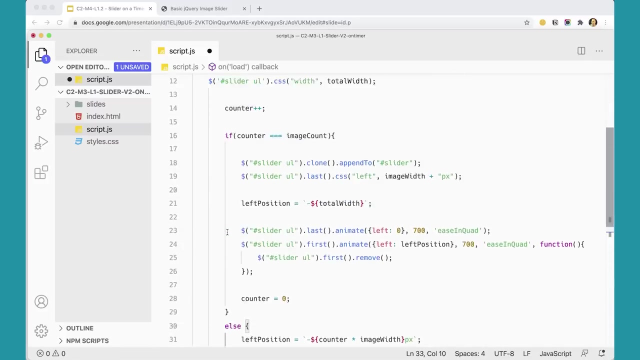 This is closing our window on event handler for when the page loads, So we want to keep that, Okay. So now I'm left with just the guts of my, of my next link thing here. I've got just the guts of that there. 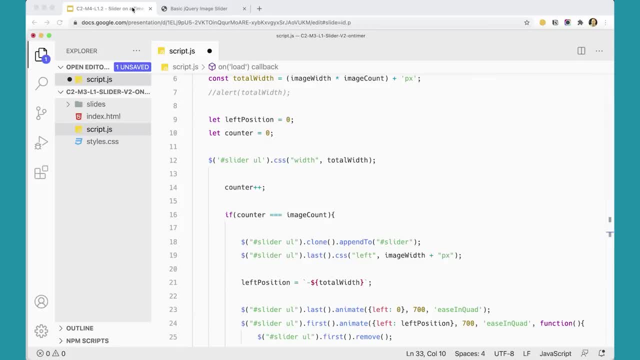 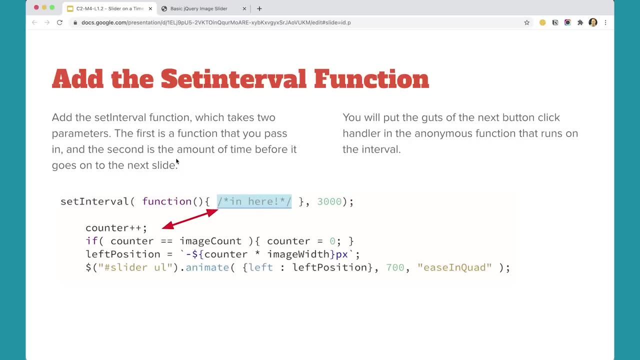 So the next thing I need to do here is create my function. that will create my set interval. I'm going to use set interval for this, but you could also use set timeout with recursion if you wanted to, But I'm going to use set interval here. 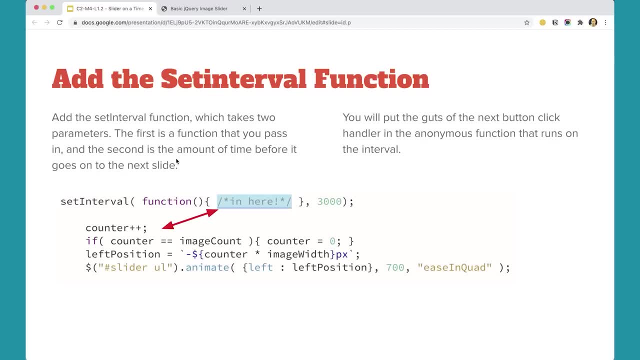 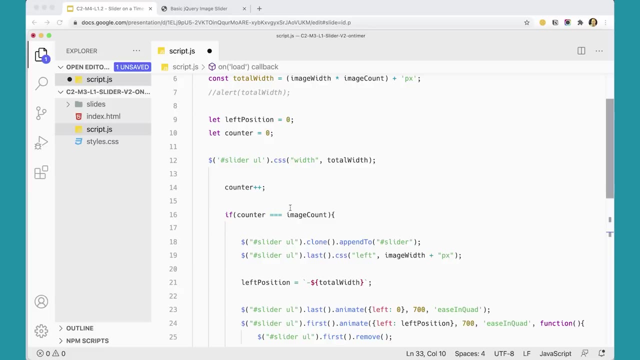 So I'm going to go ahead and add my set interval method and pass in the anonymous function and set it to 3000 milliseconds. three seconds Seems long enough for slides, So let's go ahead and put that in. So I'm just going to put it here. 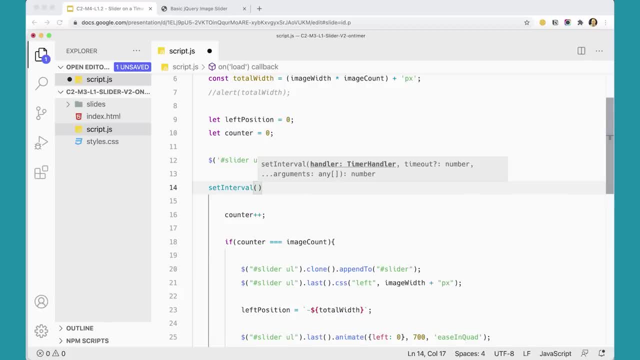 Set interval Like that. I pass in a function Like so: Oops, Extra set of those, And then I'm going to say over 3000 milliseconds, And that will run. Then all I need to do is I need to stick the guts of this stuff inside here. 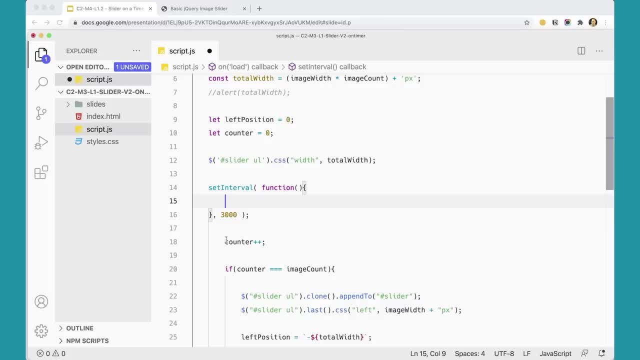 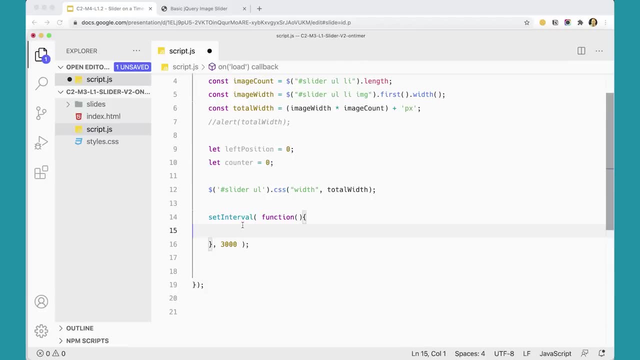 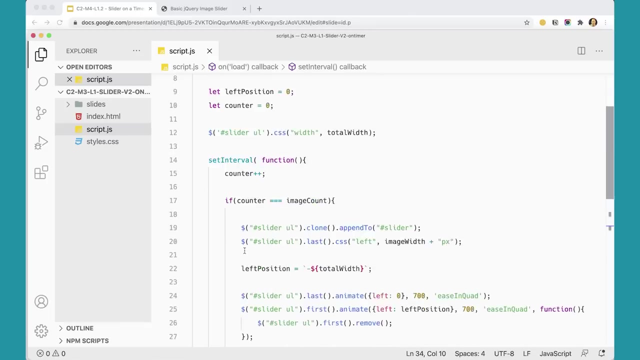 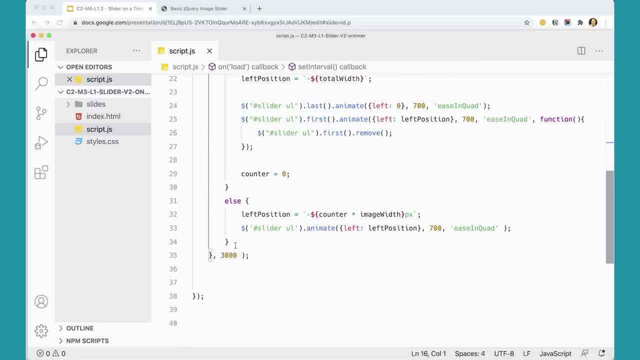 So if I move that down and then come and take all of this stuff down to here, cut it and stick it in there, That will just work. So now set interval is going to run this function And it's going to do the counter and then it's going to check my if statements. 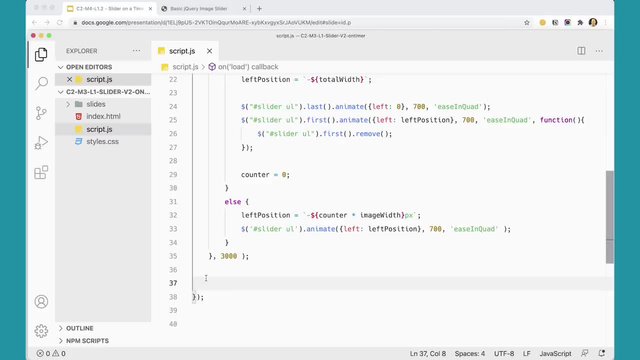 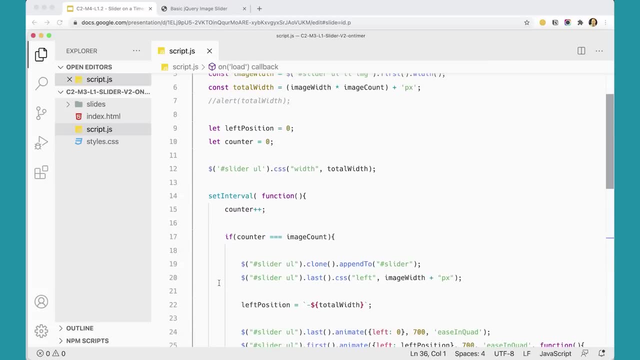 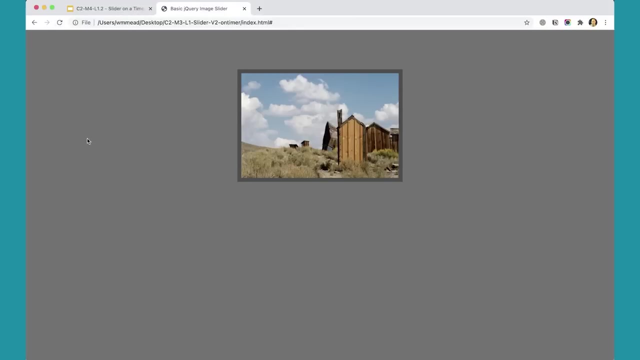 And it's going to do this every three seconds, so that it will move the slides forward every three seconds And when it gets to the end of this slide deck it'll wrap around to the beginning. Let's test it: Have to wait three seconds for the first one to go And there it goes. 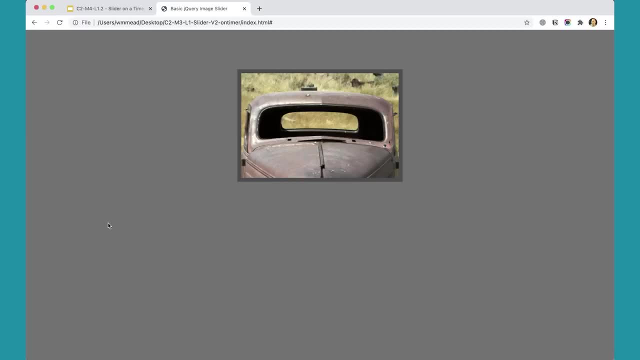 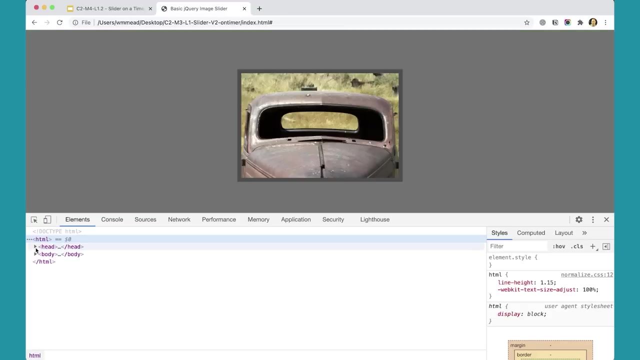 And here we are in the last slide and it should wrap around to the first slide. If you inspect And look at the body here, Look in the slider, You'll see the unordered list is moving along and changing its position here And when it gets to the end. 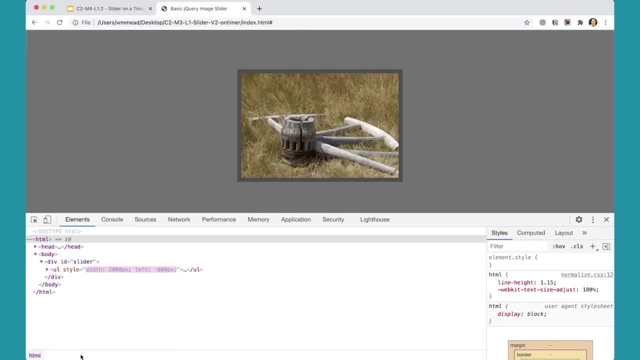 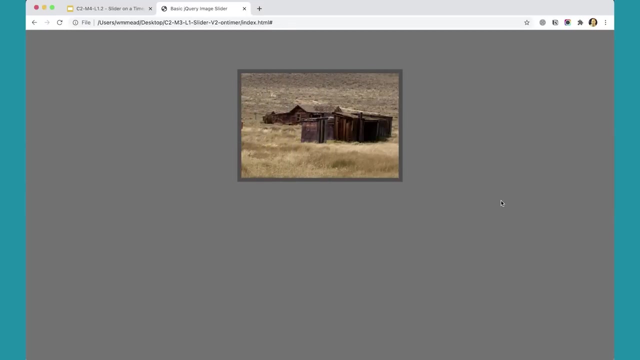 it's going to start moving, And then it's going to start moving. You'll see, the new one gets added in, moved into place, and then the old one gets taken out Right there. So that's working perfectly. Great, We got that. Now think about what you could do to make it work so that, if you hover over this, 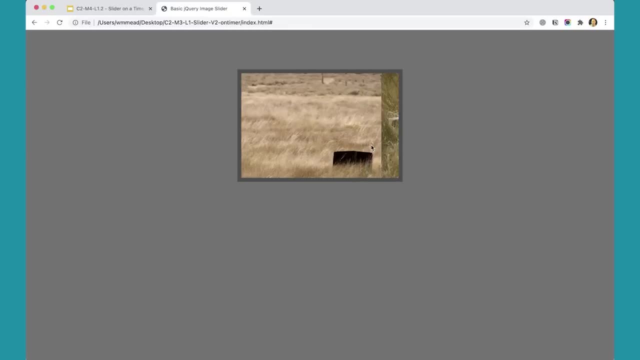 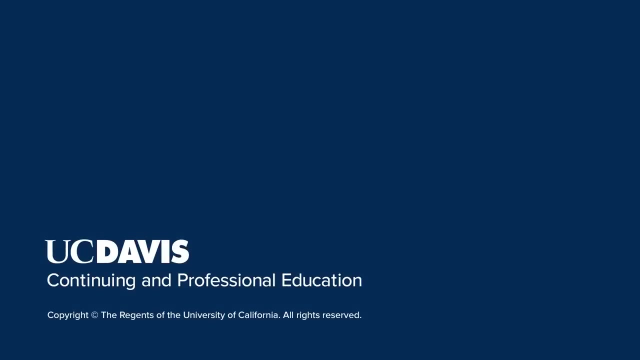 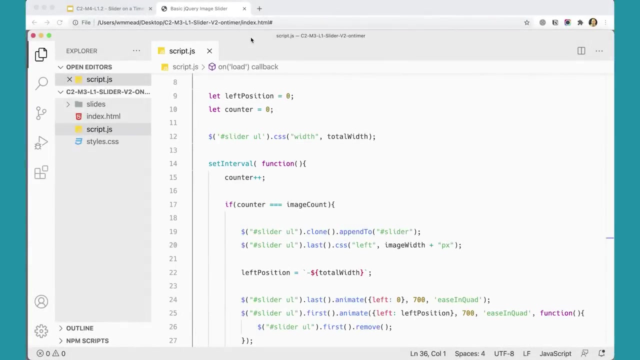 it'll stop sliding the slides while you're hovering your mouse over the slider. That's your next challenge. Did you successfully complete the challenge? Remember again, the challenge was to make it so that, when the mouse hovers over the slider, the slider stops. So let's see if we can actually make. 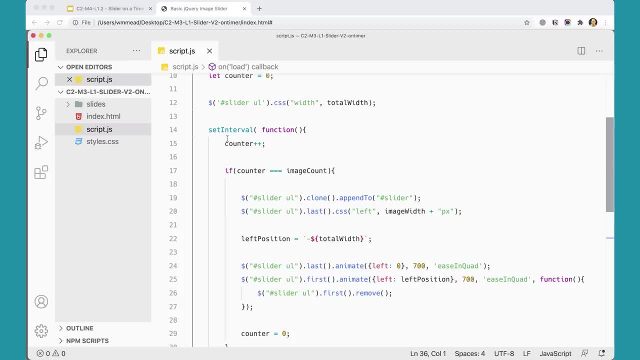 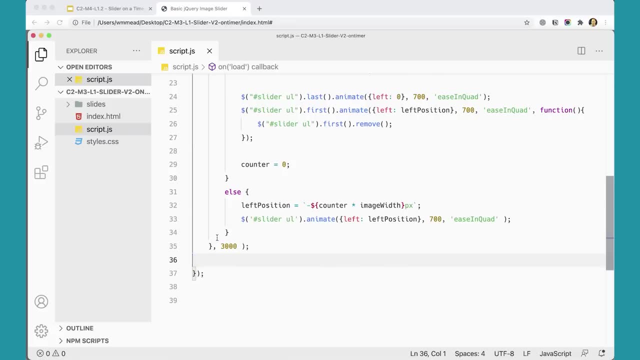 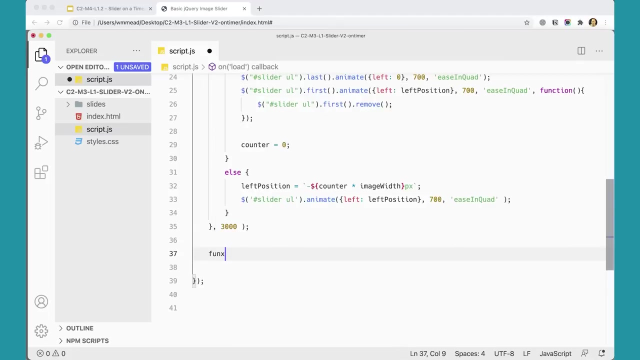 that work. What I'm going to do here is, currently I have set an interval running this anonymous function, And it runs it over 3000 seconds. What I'm going to do instead is I'm going to make a function down here, A function called slider, And I'm going to put the guts of this anonymous function. 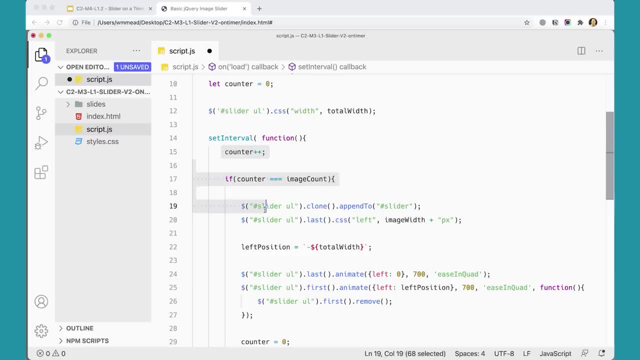 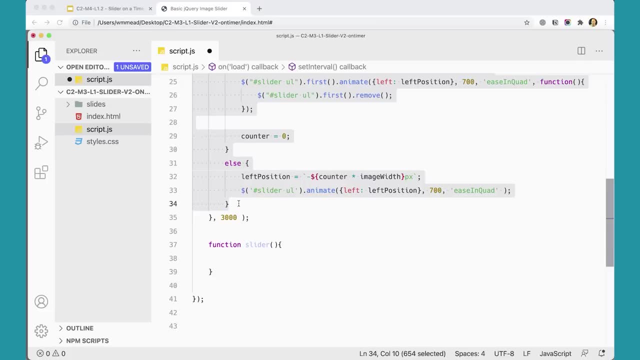 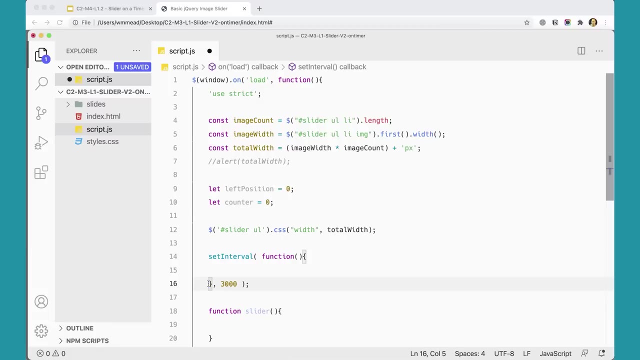 this one here inside of that function instead. So I'm going to take all of this stuff that I had moved into there all the way down to here. I'm going to cut it. So now we're back to just set interval with the anonymous function in it and comma 3000. 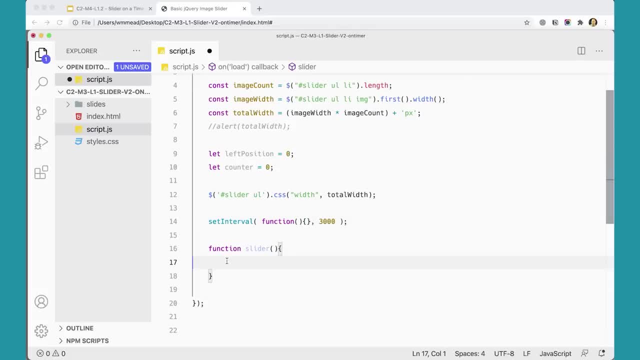 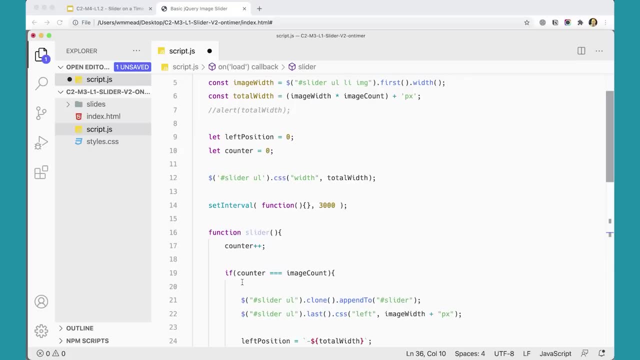 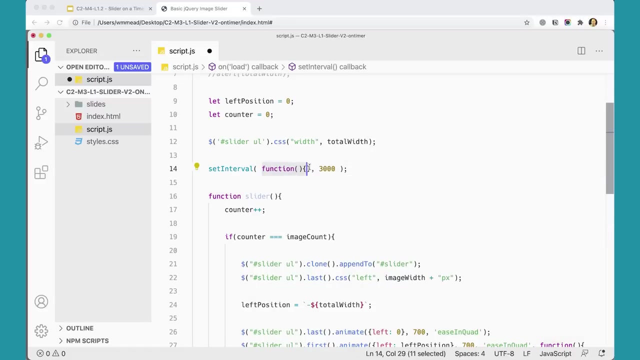 back to where we were before, But I'm going to put all that stuff in here instead, inside of this function here. So I've got my counter and all of this stuff inside of here And then here I'm going to say: run slider. 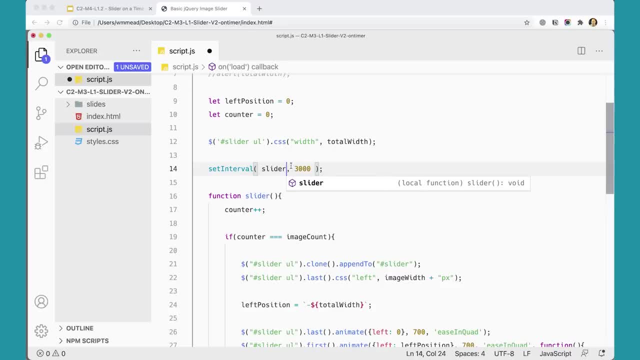 And this is a reference to my function- slider. I do not put the parentheses in here. if you put the parentheses in here, won't wait 3000 seconds, it'll just go right away. we want to wait 3000 seconds and then run slider. 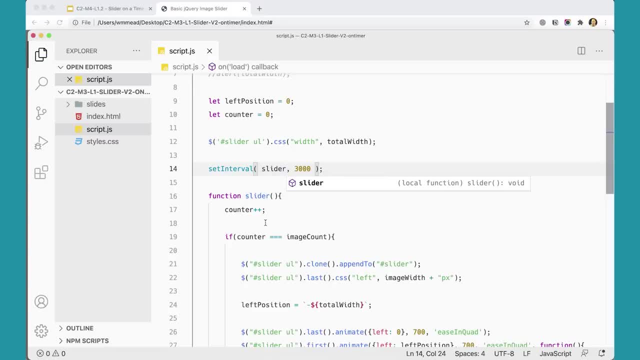 So then it's going to go find the function slider and run, And that should work in terms of exactly the same thing that we had before. this should just run. So let's just test that really quickly. If I come over here and refresh the screen, it should wait three seconds and then start. 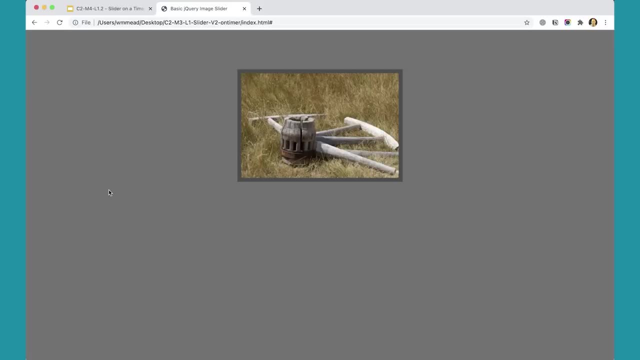 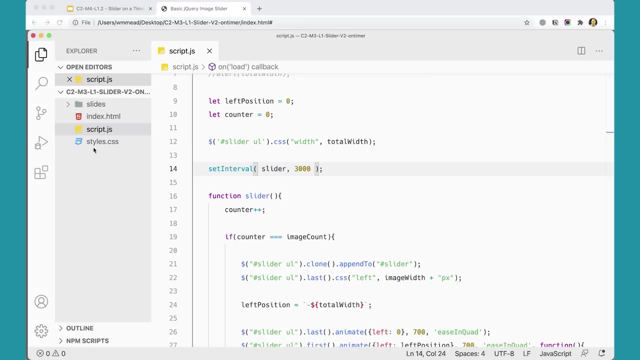 running the slider And that works the same way it did before. But the difference now is that I can now set my set interval here. I can assign it to a variable. So I can assign that to a variable. I could put: let my slider equal set interval. 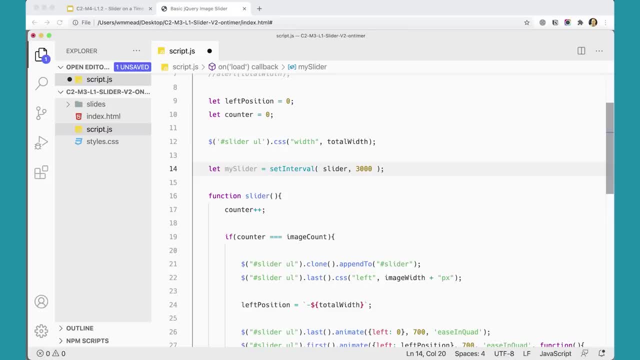 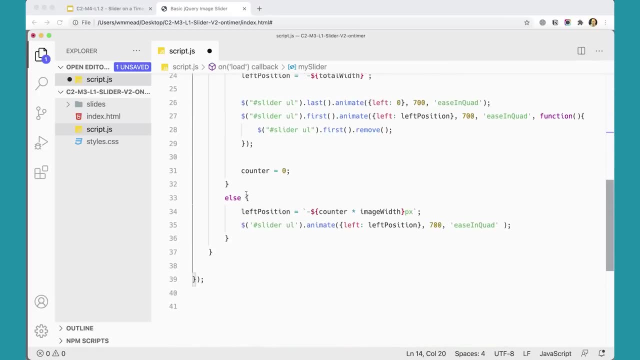 Slider And then I can actually create an event listener that will run when the, that will do something when the when the mouse hovers over it. so I'm going to make the. I'm going to make an event listener for when you hover over this slider. 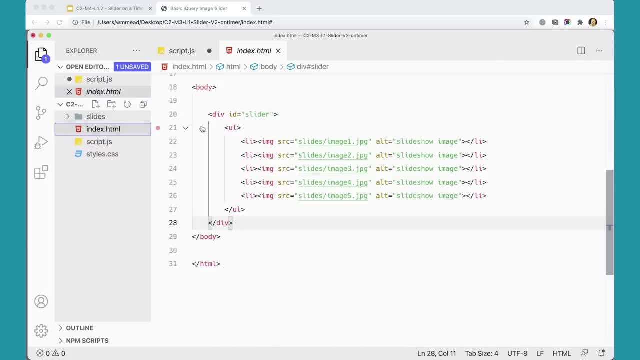 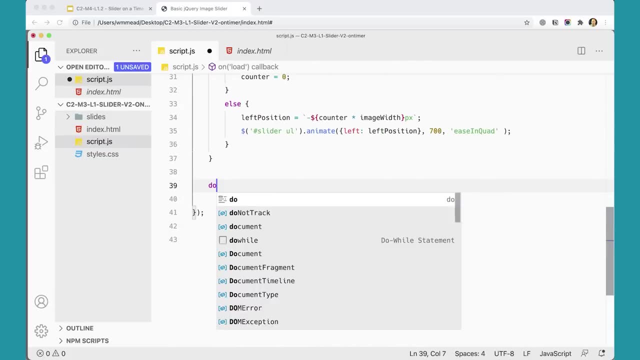 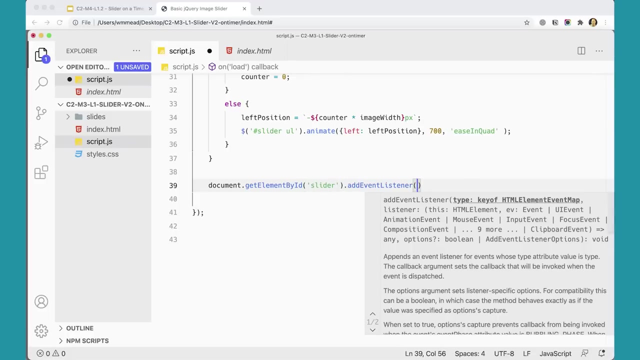 This element on my page here when you hover over the slider here. So down here I'm going to do document dot, get element by ID slider dot. add event listener And when the add event listener runs I'm going to be looking for mouse over. 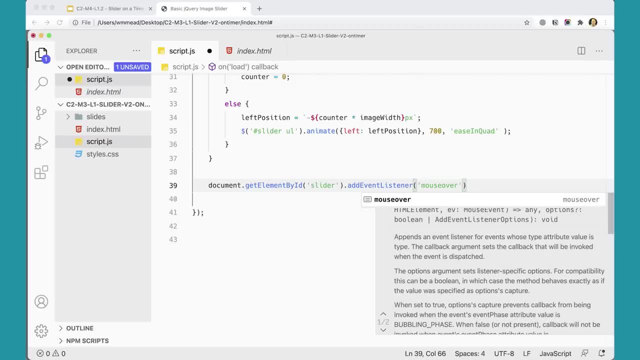 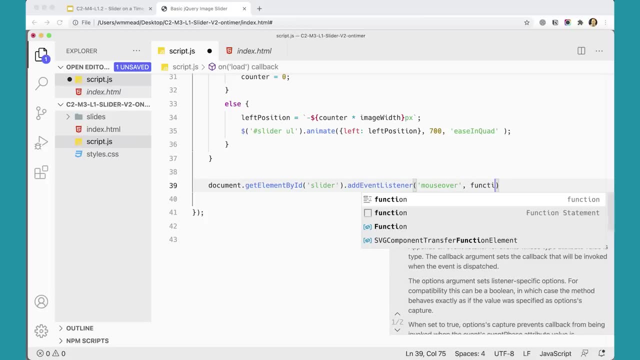 And you mouse over, I'm looking for that event And then I'm going to run a function Like: so, Extra set of curly braces. again, I keep doing that, Alright, so I'm going to run a function there When you mouse over this. 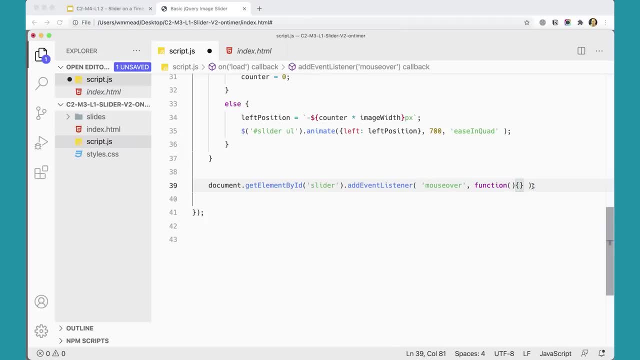 Over that element, the slider. Okay, And what function am I going to run in here? Well, I'm going to say clear interval My slider, And that will stop it from running. So that's great. So that stops it, I hope. 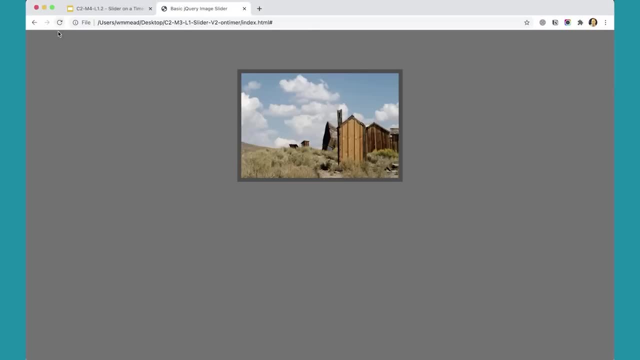 Let's test it. If I refresh this And then stick my mouse over there, It should stop the slider, It should not run anymore. So now I've cleared my interval And it's not going to advance the slides. So now I need one that will actually advance the slides when I roll off. 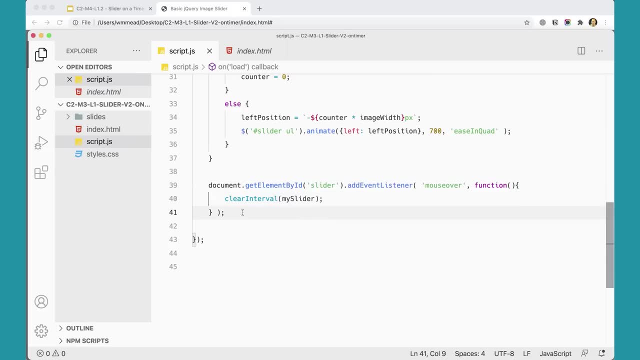 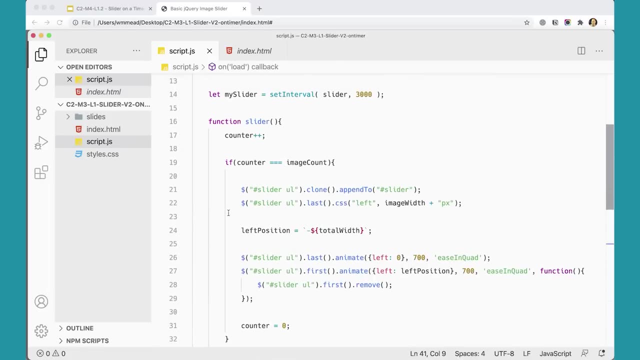 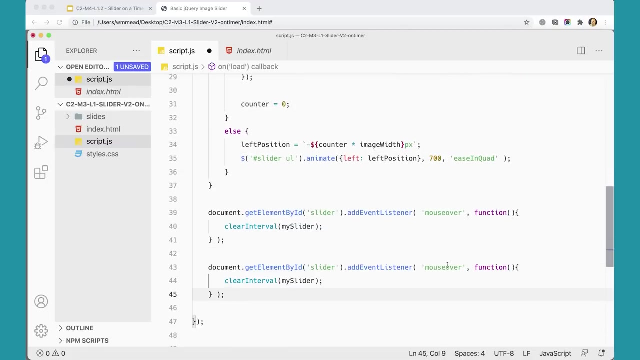 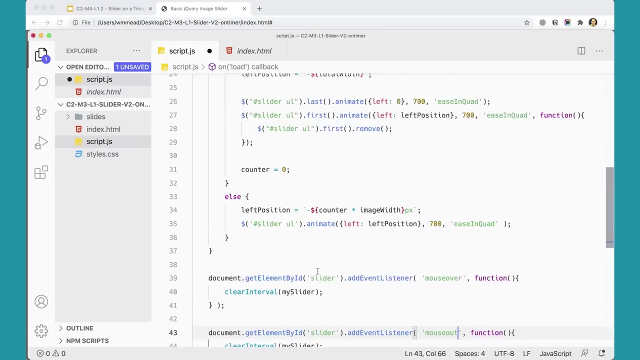 Coming back here, I can actually copy this. Okay, Okay, Yeah, Get interval slider, add Event listener. mouse out And I'm going to run a function. And what am I going to run? I'm going to say Slider. 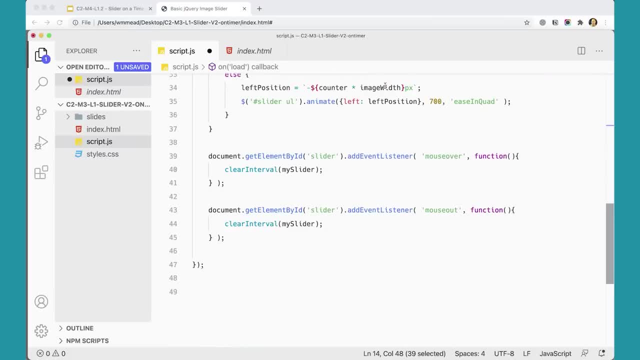 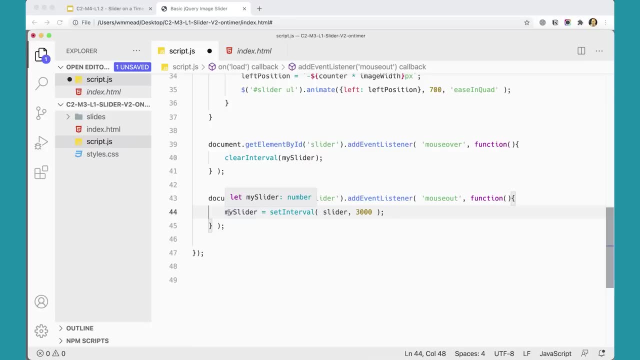 I'm going to just do this again, So I can actually just copy that. This is why I used let up there instead of const. Just because I'm reassigning this variable, In order to reassign it, I need to be able to set it to let up there. 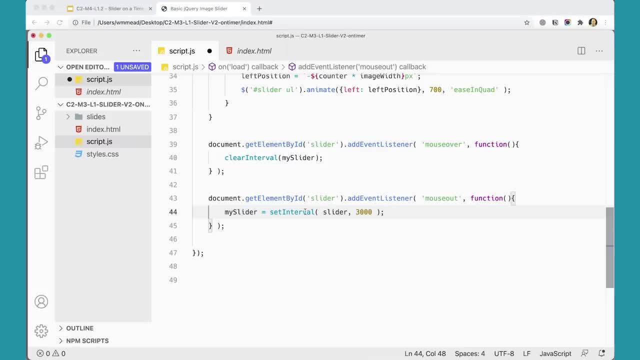 So now, if I set that to set interval slider, When I mouse out Slider is now going to have set interval on it again And that should run. So let's test that and see, Come back here and refresh it Now if I wait three seconds. 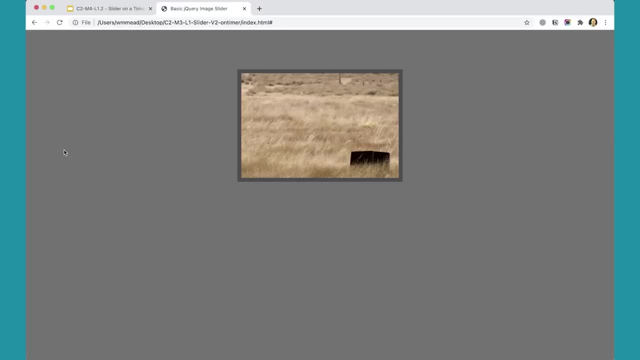 My slider should start going And it does. If I roll over the slider It should stop. So now Set interval has been cleared And it's no longer Picking up, that It's no longer advancing the slides. But then if I roll off of it, 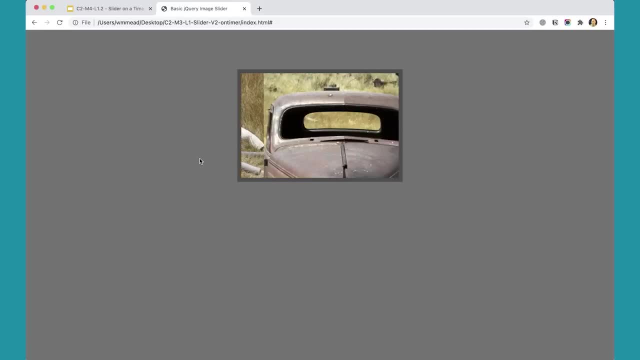 And wait three seconds. It should start back up again. Look at that. It's working perfectly. So hopefully you were able to solve those two challenges. If not, I recommend going through this a few times. Do it on your own a few times. 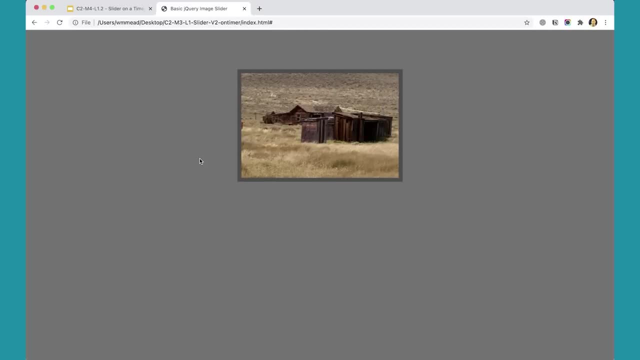 Create your own slider Or create your own script Where you can play around with set interval And set timeout. Another thing to try is: I'm using set interval here, But could you do the same thing with recursion And set timeout instead? 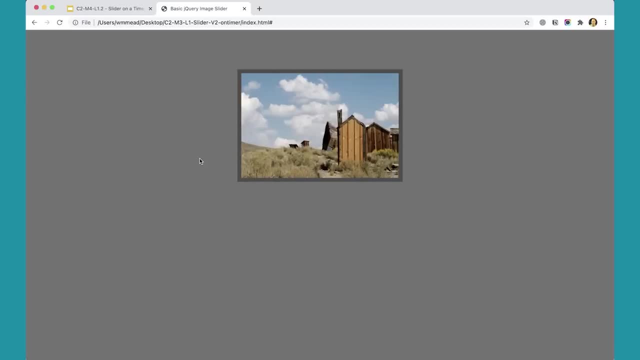 That would be an interesting thing to try to do. So The best way to learn JavaScript Is to keep practicing with it And to keep challenging yourself By making small experiments, Taking a small script that you have And then extend on it. 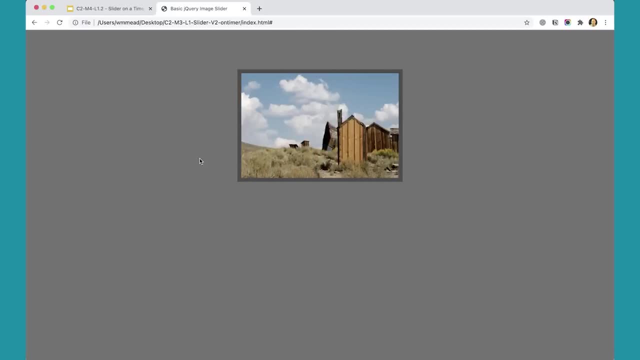 And see if you can make it do a little bit more. What else could you do? Could you make it so that It has the buttons For advancing the slides manually, But it goes automatically When you're not using the buttons, But then when you do use the buttons? 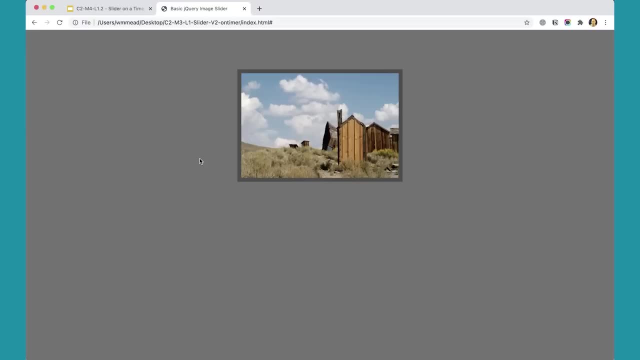 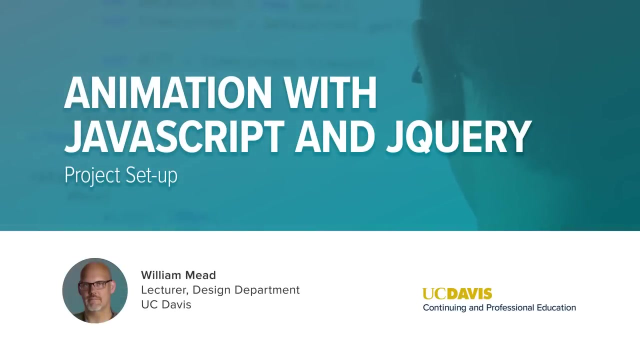 It moves it manually. That would be an interesting Modification to the script. Maybe you could come up with other ideas And other things that you could do In this project. We'll look at creating a content rotator. It will use jQuery. 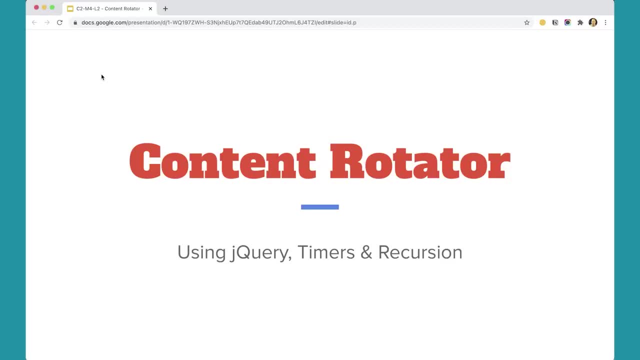 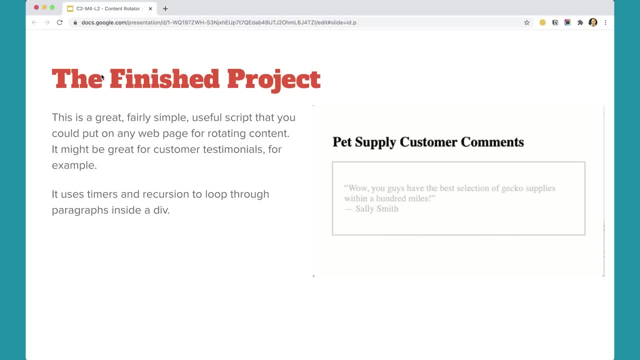 It will use timers And recursion. This is a fun project. I hope you enjoy it. It will give you a quote That rotates around To different quotes After a period of time, And this is potentially very useful. You could put this on a website. 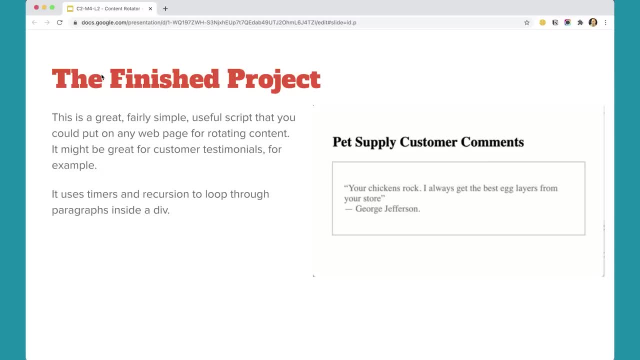 To rotate customer testimonials Or that kind of thing. In fact, I came up with this script. I wrote this script myself Because a client needed, On his website, To make something that rotated testimonials. And this is, I wrote this script. 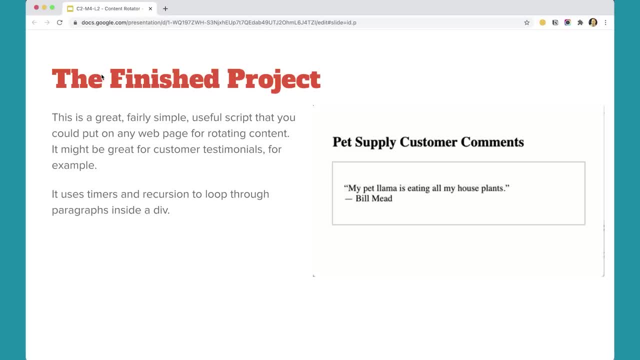 In the early 2010s, So a lot of these scripts Hadn't been written, Were easily accessible At that point, So I had to write one myself. It was kind of fun to do, But I really enjoyed putting this script together. 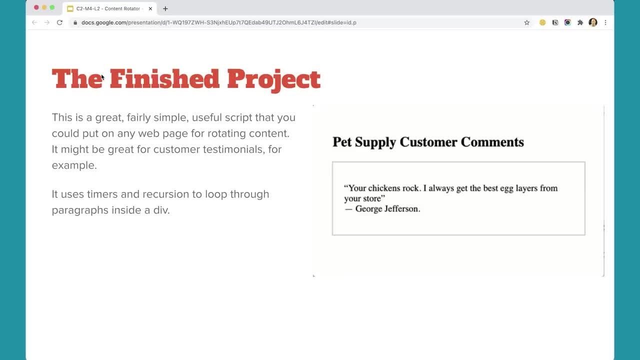 The website I was building for him Was in WordPress And I wanted something super simple That he could just put in paragraphs And they would just automatically Get rotated around. It was kind of a fun, Simple little project And it generates a project. 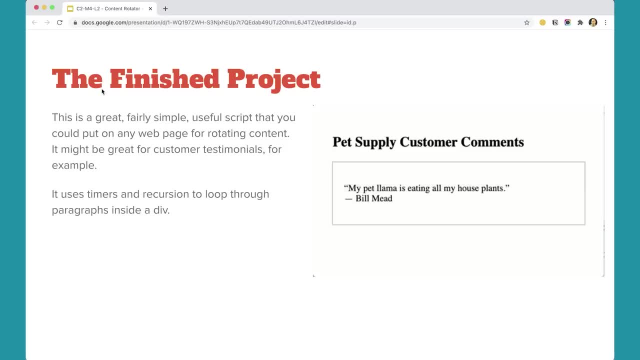 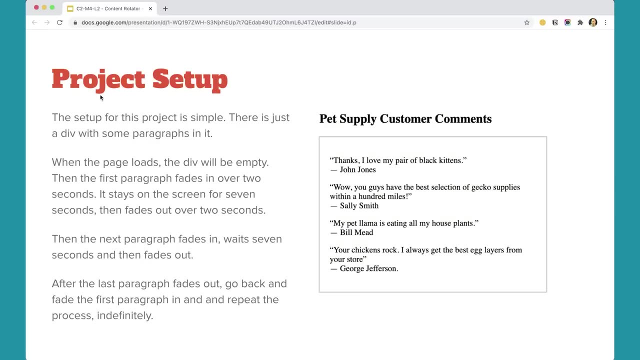 That you could use for lots of websites. So let's take a look At how this is set up So we can actually work with it. The project setup is really simple. We have a page With a div With four quotes in it. 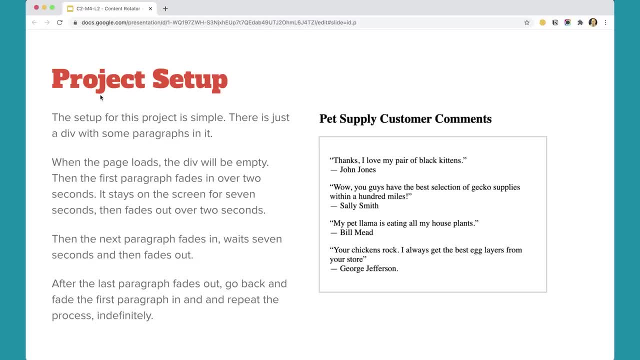 And you could add quotes Or remove quotes And put in more if you wanted to, And basically They're hidden, And then So that the div is empty to begin with, Then the first paragraph Fades in over two seconds. 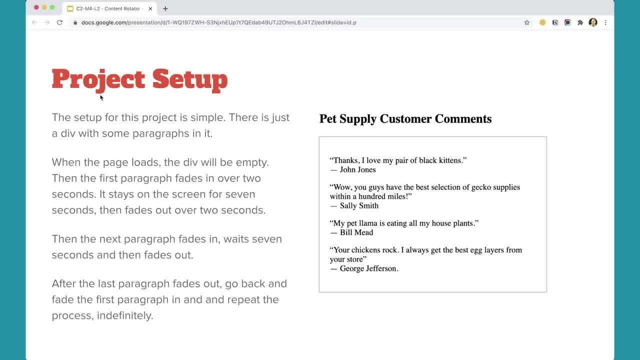 It stays on the screen for seven seconds So you can read it, And then it fades out over two seconds. Then the next paragraph fades in, Waits seven seconds And then fades out. After the last paragraph fades out, We want to go back and fade in the first paragraph. 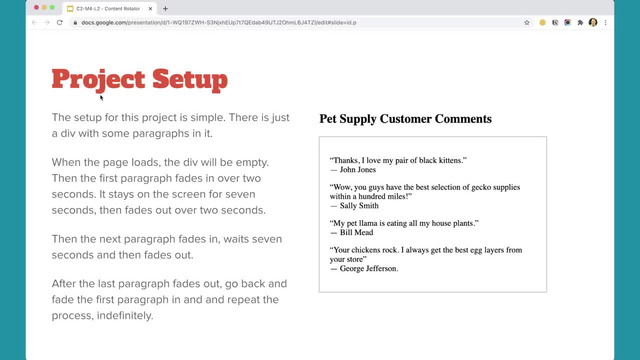 And repeat the process indefinitely. This is a really great job for recursion. We'll also be making use of the jQuery effects library a little bit Along with some of the other features we've talked about in this course, So I hope you have fun with it. 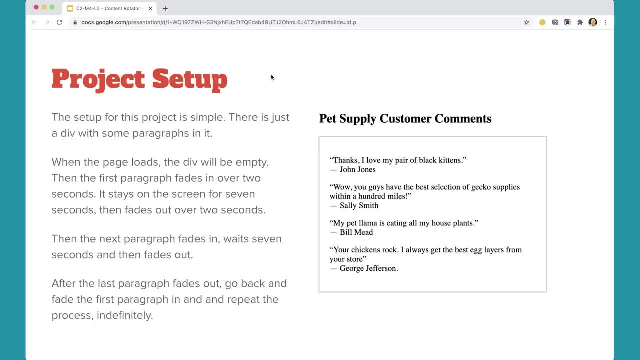 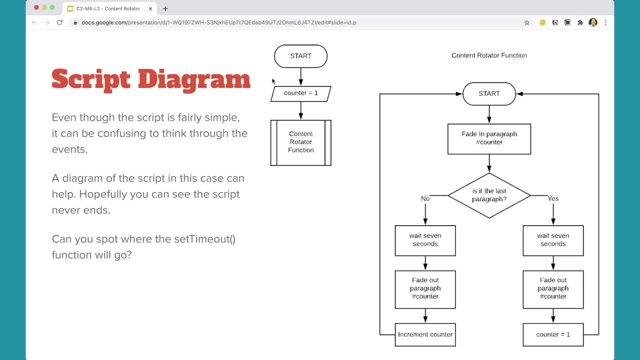 And end up with a script that you can use for something It's pretty fun To start with. Recursion can be hard to wrap your head around. It can be really hard to think about Trying to puzzle it out And make it all work. 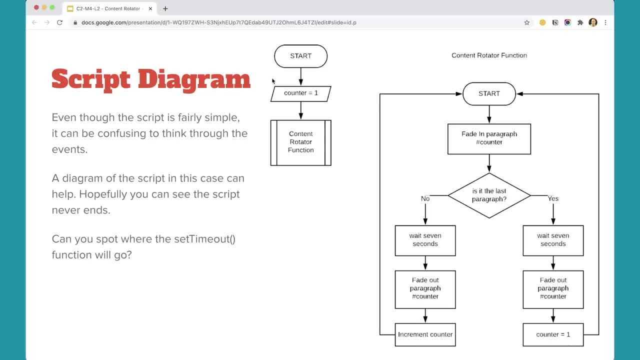 So I have here this diagram that can help us Sort of simplify it And think about exactly how this is going to work. So when the script starts It's going to set a counter to one And then it's going to run a function. 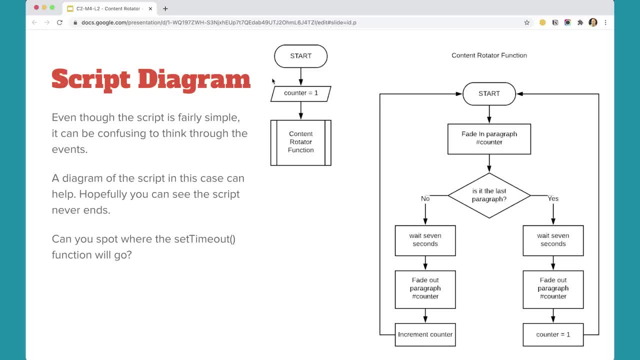 Called content rotator. And then on the right here I have that function, Content rotator, And it starts. It fades in the first paragraph Or it fades in paragraph that matches the counter number. To begin with, It's counter number one. 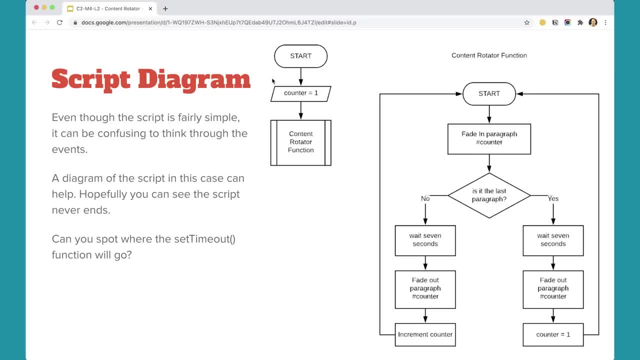 And then it asks: Is it the last paragraph on the page? If it is, Then we're going to wait seven seconds. Fade the paragraph out And set the counter back to one. If it's not, Then we're going to wait seven seconds. 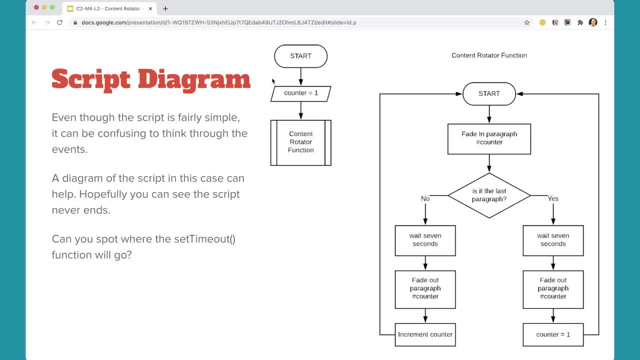 Fade the paragraph counter out And then increment the counter, And then we run this function again. We run content rotator again And that's where the recursion comes in. So this function is going to call itself And will be using Set time out. 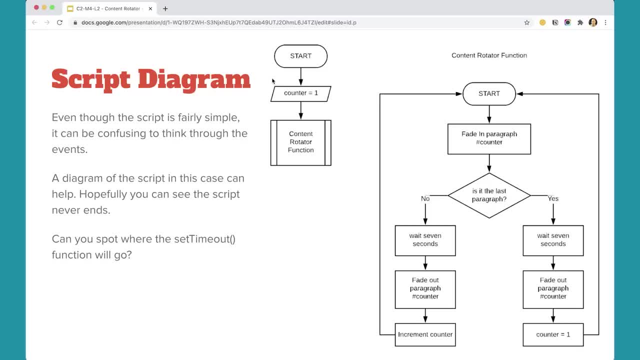 So can you spot here Where set time out happens? We're going to fade the paragraph in And then we're going to wait seven seconds. So there is a set time out Where we wait for seven seconds And then we're going to fade the paragraph out. 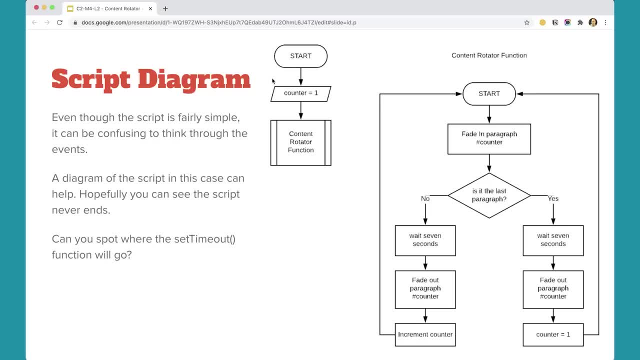 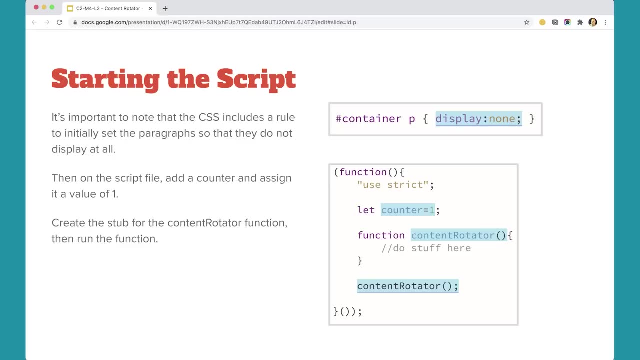 And then we're going to wait for seven seconds And then we're going to fade the paragraph out. so that's where the set timeout will go, is when we're waiting seven seconds. let's get started on the script. the first thing to note on this script- and I 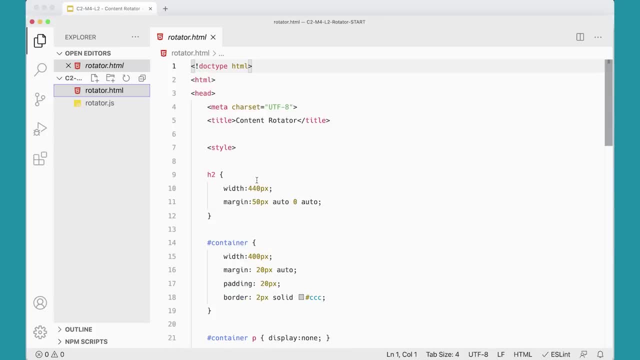 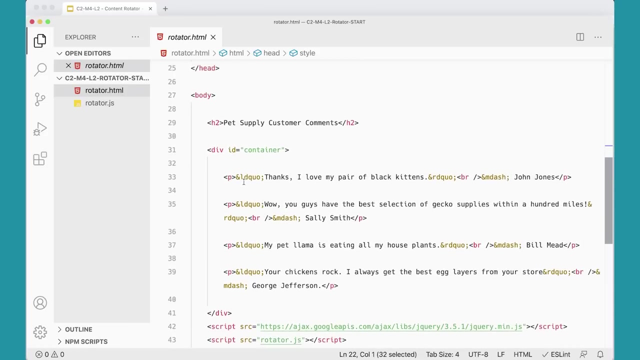 have my files open here in Visual Studio Code here and the first thing to note is that in the CSS I have all the paragraphs inside my container. so here's my div ID container. they're all set to display none. now when you look at this it might look a little bit weird because of these things here, but this is just an. 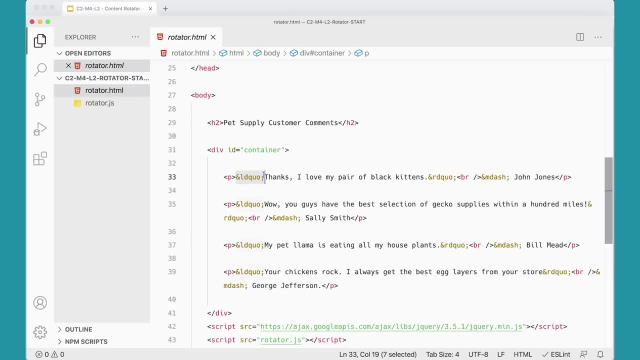 HTML entity that's creating a curly quote. so that's the left double quote, and then this one over here creates the right double quote, and then this one in here creates an em dash. in design, typography is very important and rather than just I could just put this straight up into. 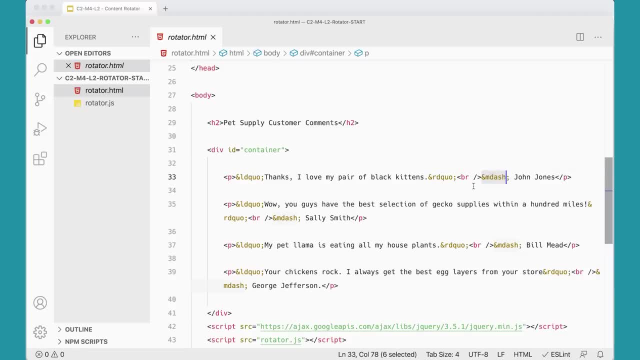 down quotes, but those don't look as good and since I want this to look a little bit nicer, I'm putting in the curly quotes and the em dash, which is the longer dash, rather than the end dash or the hyphen, and if you take it, take a. 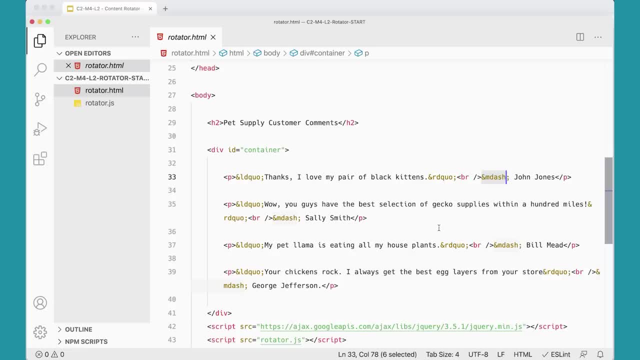 typography course. at some point you'll learn all about these different glyphs that are in or that we can use when we're creating content. the quote button on the American keyboard, anyway, can handle it really represents six different possible characters. there's the straight up and down double. 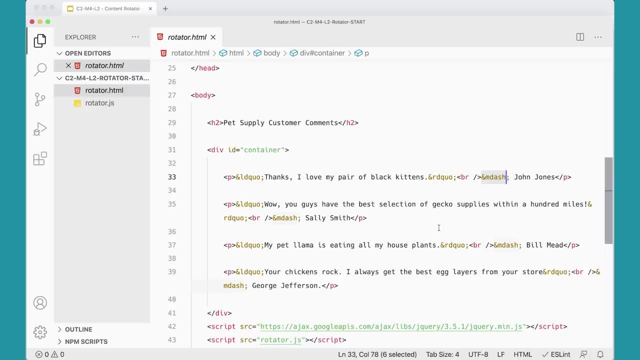 quote: the left curly quote, the right curly quote, and then the same thing for the single quotes. there's a straight up and down single quote: left single curly quote and right single curly quote. so that's six characters and one key, and other languages may apply to that. so that's the straight up and down double. 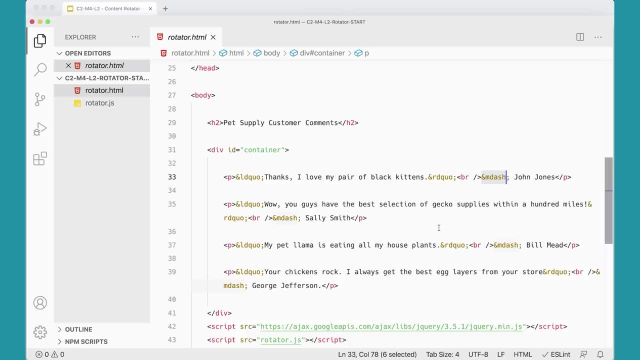 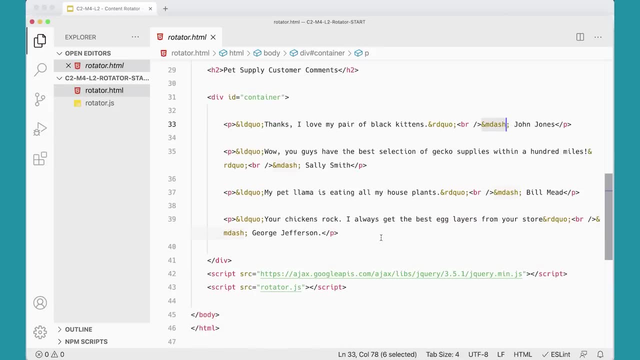 quote or any legal Korean characters associated with that as well, but for English it's actually six characters, okay. so we've got that all set up. we have our jQuery library loaded down here and we have a script, a rotatorjs, and that's where we're going to do. I offer here is: on the rotatorjs, we've got our 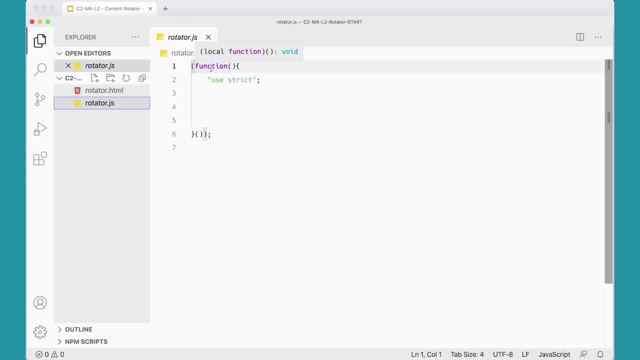 II, f, e are immediately invoked. function expression set up to keep everything out of the global em and I can also. I have here in the data center that's a linear anaerobic function and it'll also be used by the program and in the build process. 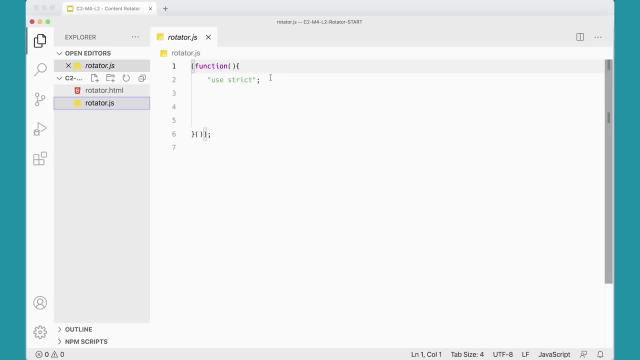 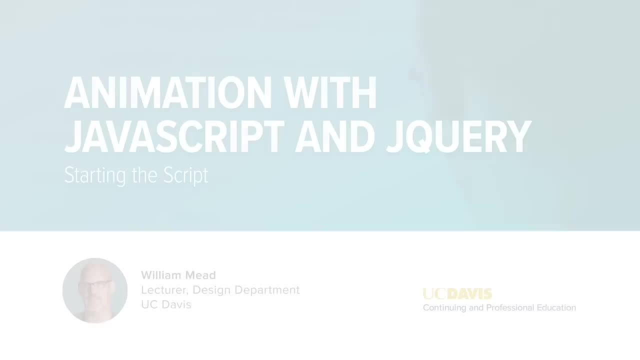 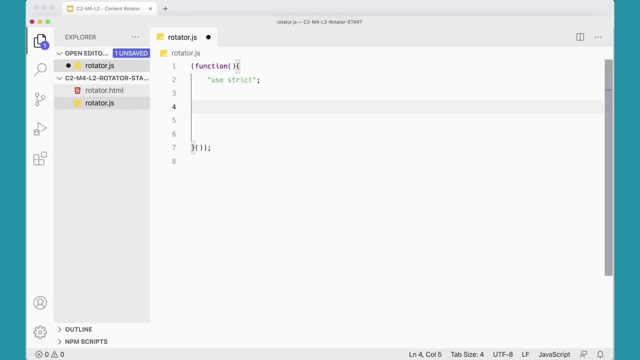 global scope and we've got our use strict directive in there. okay, we're all set and ready to start working on our script. here we go to write our script and get our content rotator to work. first thing i need is a variable, let counter, and i'm going to assign it the value of one. 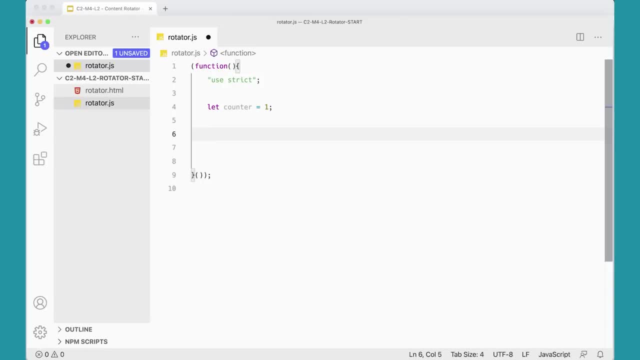 and then i'm going to make a function called content rotator, like so, and we'll do stuff in here, do stuff, and then i'm going to call that function content rotator to get it started and make it work. there we go. so this will get us started with our script. 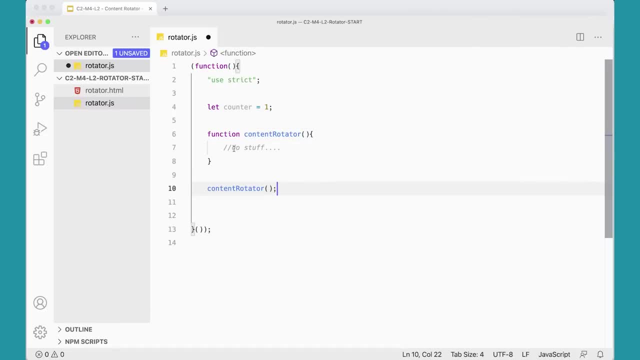 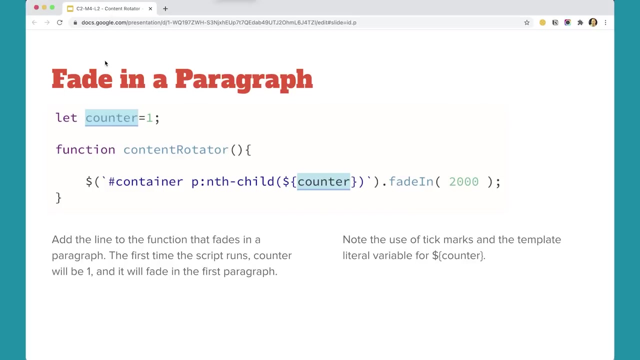 with our function and our counter or variable and we'll gets our file all set up and ready to go properly here. our next job is to get our first paragraph and fade it in. we'll use our counter to do that and the css nth child filter to allow us to get the first paragraph, because remember. 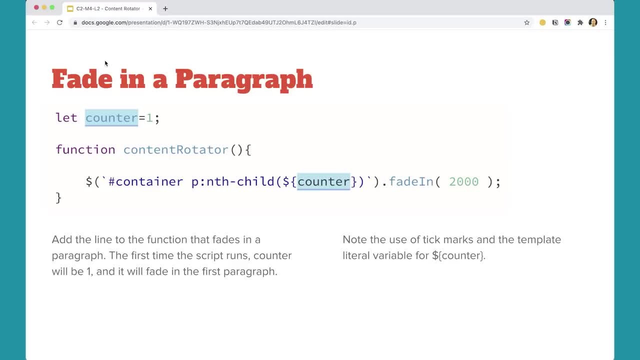 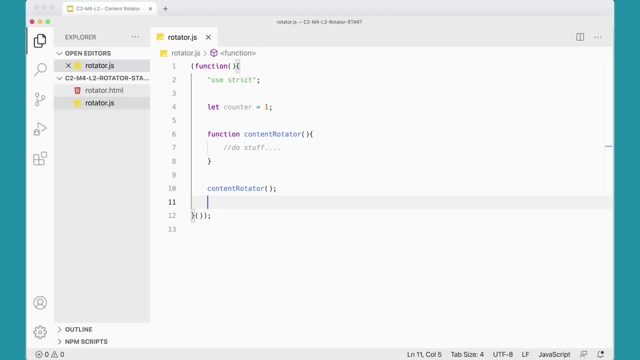 currently all paragraphs are set to display none, so we can use our jquery object to go get that first paragraph and fade it in. so let's do that. so down here inside content rotator, here we want to do, we want to use our jquery object to go get- i'm going to use my tick marks to- 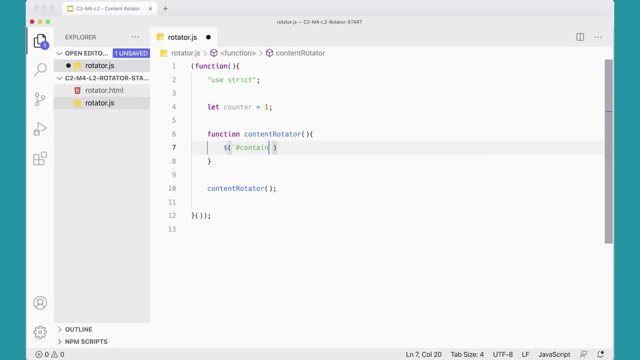 say: pound container, p? nth child parentheses. now, if i were to put a one in here, that would go get the first paragraph. if i were to get a two, i would get the second paragraph, i would get a third paragraph, so on and so forth. you might wonder why i didn't start my counter with zero, and frequently 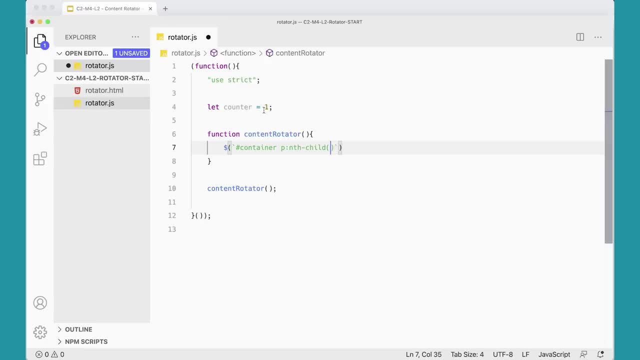 we do when we're working with arrays, because the first element in the array is zero, indexed, But the nth child pseudoselector is actually indexed with one. So one will get me my first paragraph, But I don't want to put a one in there. 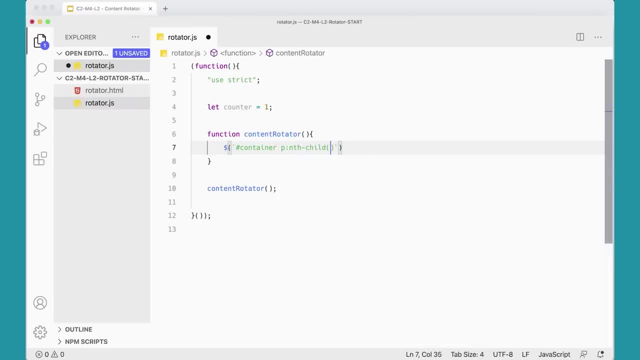 I want to put the variable counter. So I can do my template literal, like so, and put the word counter And that will go get counter, which is a one in this case, the first time this runs. So that goes and gets that first paragraph and gets it in there. 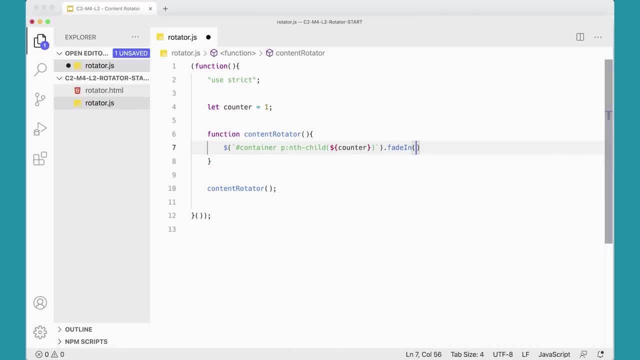 And then we can do fade in 2,000. Because, remember, this is our jQuery effects library here, So we can actually fade in that first paragraph there. Save that And I'm going to come over and give it a try over here. 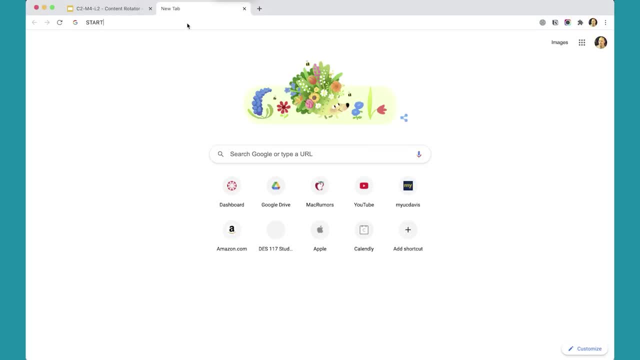 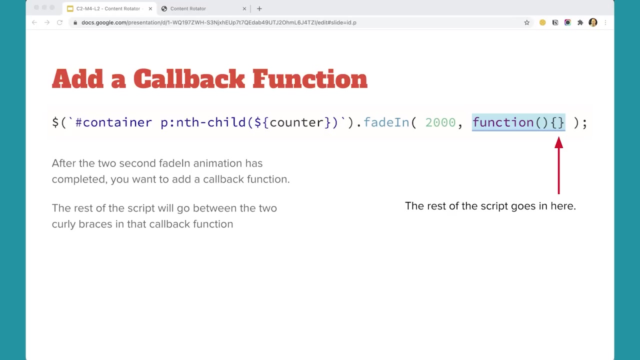 Oops, that's not what I meant to do. Open this file here. When I open it, it fades the paragraph in Great. So that's working perfectly so far. Now that I've faded the paragraph in, I need to wait seven seconds. 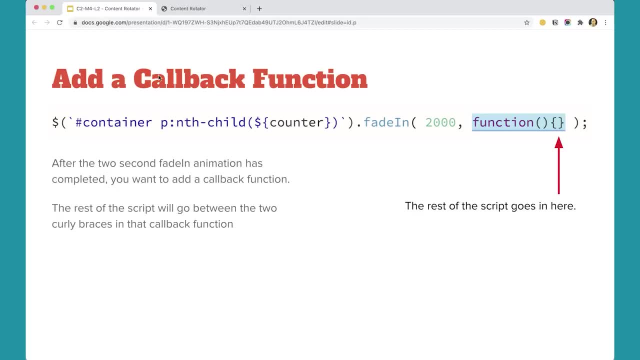 And this is going to happen after the two-second fade in Remember, with jQuery we have a callback function that we can use with our fade in helper method. that will allow us to do something after it has faded in. So after that animation has run, we want to run that callback function. 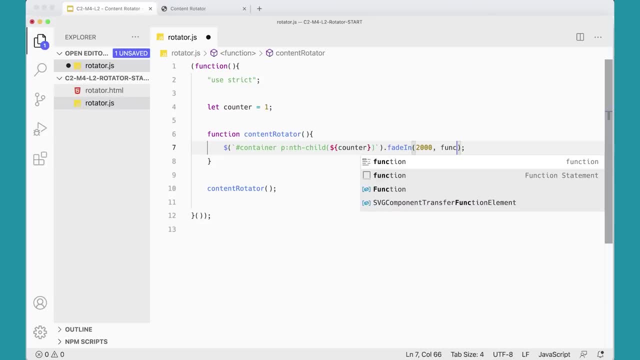 So fade in comma function. We want to run this function after the fade in is complete, And that's where we're going to put the rest of our script. It's going to go between these two curly braces here. Everything else we do is going to go inside this callback function. 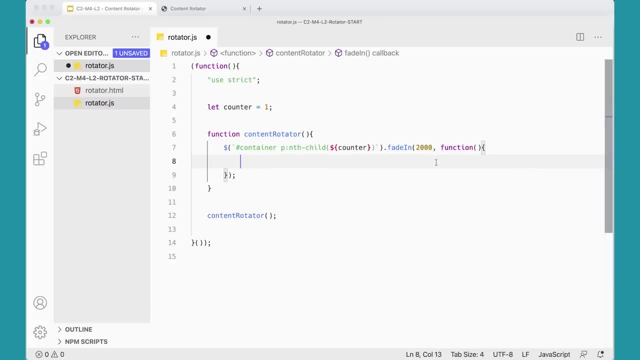 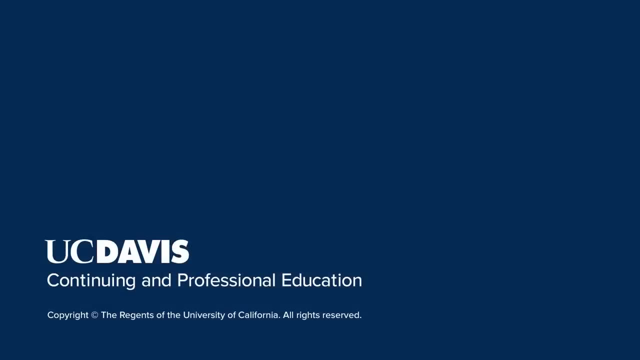 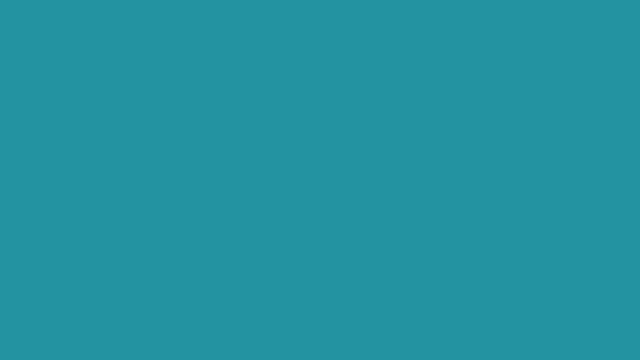 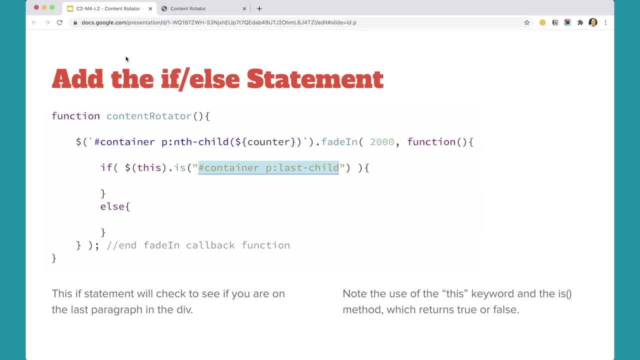 So after we fade it in, we're going to run a function And in that function we'll set it to wait. So we're going to wait seven seconds and then check to see if we're on the last paragraph or not, Now that we've faded in the first paragraph, and after that two-second fade in has taken place. 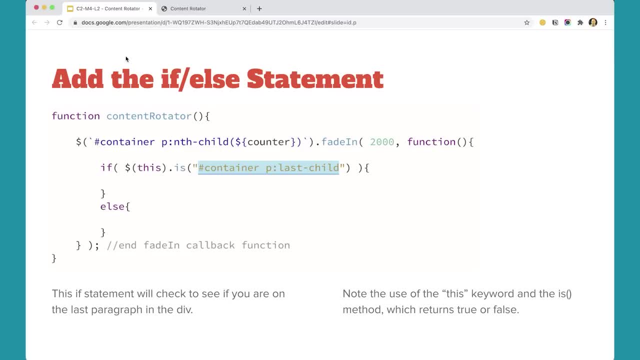 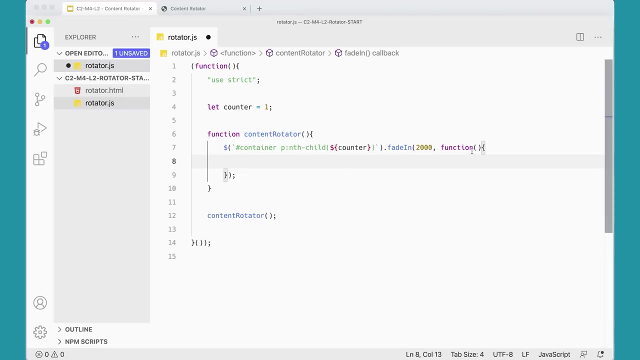 we're going to run a callback function And inside that callback function we're going to check to see if this is the last paragraph or not. So let's get that if statement in place and then we'll go forward from there. So we've faded that in. 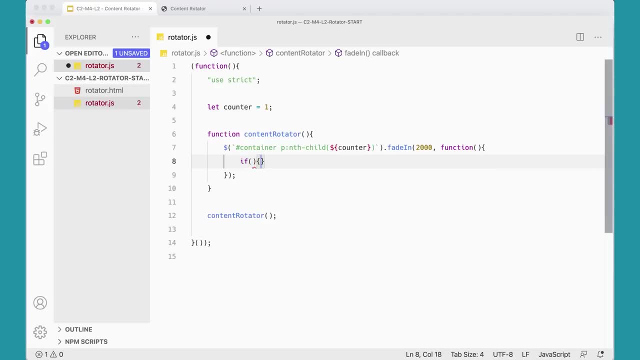 Now we're going to do an if, If, parentheses and we'll do something in there. And then we've got an else where we'll do something in there. Okay Okay, Do something, Do something else, Okay, If. 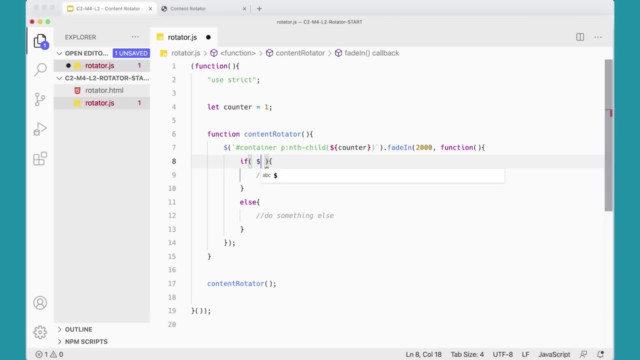 And what am I checking? I'm going to use my jQuery object and the this keyword, This, This paragraph. If this is- Oops, that's not is, Is There we go. Is Is a jQuery. Is a jQuery function that will return true or false. if something in there is true, 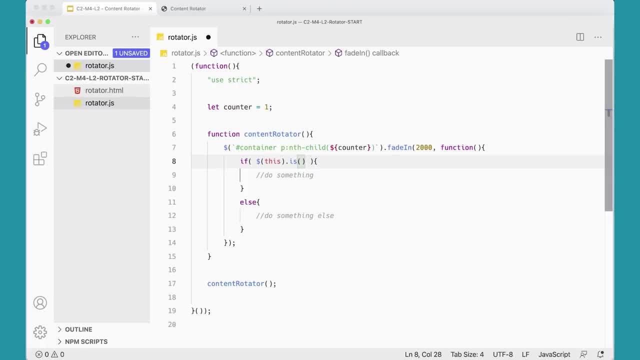 So if this is, and then I'm going to say, if this is in here And I can't remember, do I need to get my jQuery object for this? I don't think I do. I think I can just put quote: pound container. 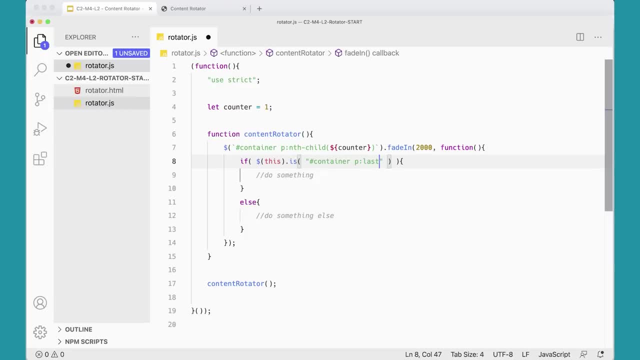 P, colon: Last Child. Is it the last one? Is it the last paragraph? I think I've done that right. We'll test it in a minute here, But it looks like I've got that right. Okay. so if it's the last child, we're going to do something, and then, if it's not, we're going to do something else. 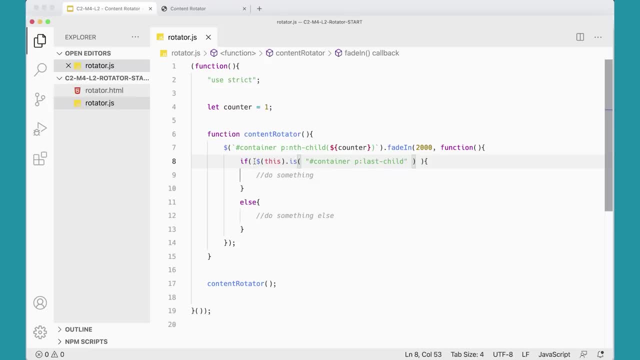 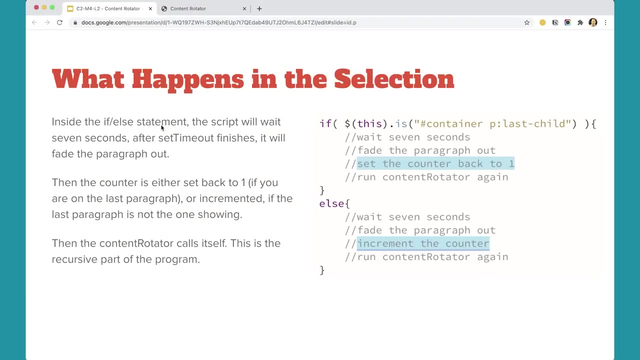 What we're going to do is wait seven seconds and then run the content rotator again or reset, and also increment the counter or reset the counter. Let's go back over to our slides here. So, yeah, we're going to wait seven seconds, fade the paragraph out, set the counter back to one and run content rotator again. if we're on the last paragraph, 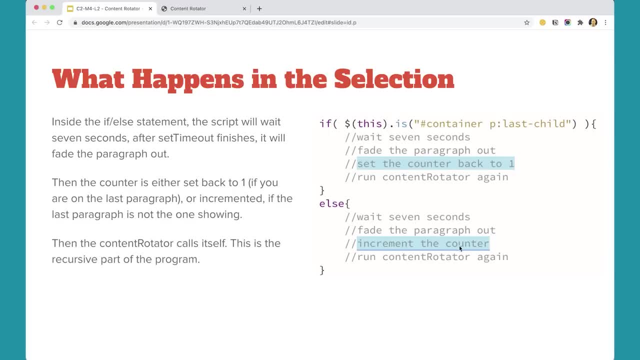 If we're not, we're going to wait seven seconds, fade the paragraph out, increment the counter and run content rotator again. So the only real difference between these two is what happens with the counter, and hopefully that makes sense And also you'll see here where the recursion is taking place. 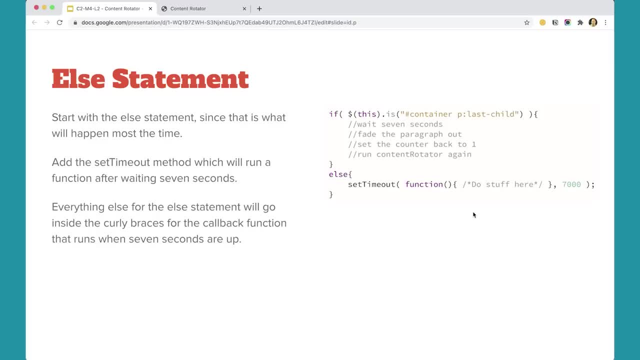 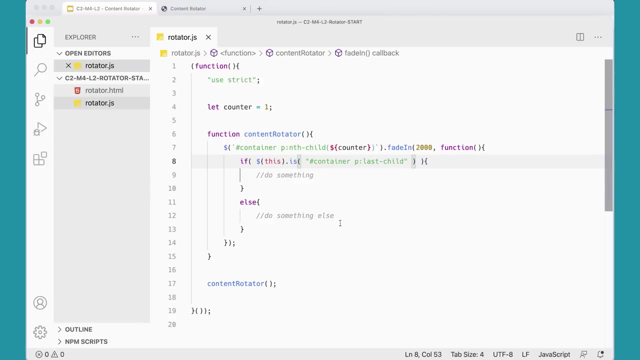 So let's work with the else statement first, because I think that one's a little bit easier. So let's add the setTimeout function in there and then we'll go forward with that. So down here we're going to say setTimeout and that's going to run a function after setTimeout. 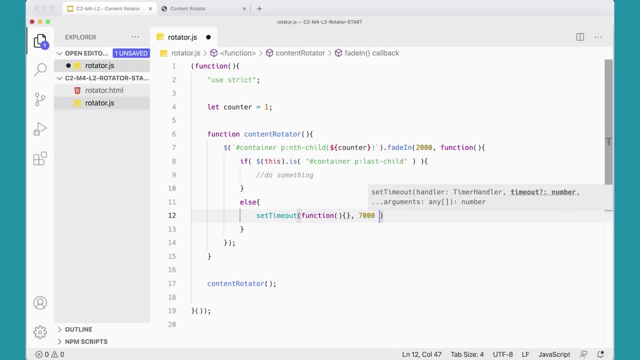 So we're going to run a function after seven seconds- and I like to put a little extra space in here just to make it so it's really clear what's going on there. So we're going to run a function after seven seconds and then we're going to put the next piece inside here. 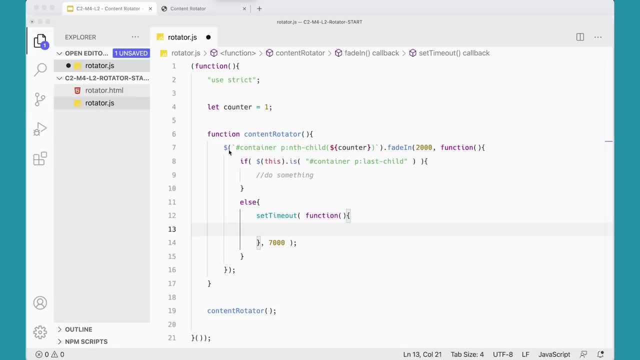 So what we're going to do is, after seven seconds, we're going to run a function after setTimeout. So after seven seconds, we're going to take this same thing here and just copy that, Come down here and paste it. 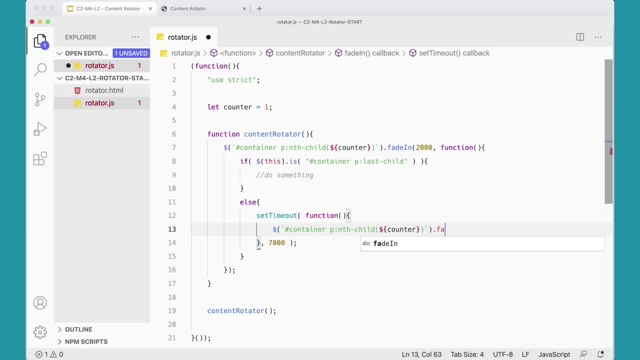 We're going to take that same thing and we're going to run fadeOut over two seconds And that will fade that paragraph out after seven seconds. So now, when the content, When the content rotator starts, it checks to see if it's the last child. 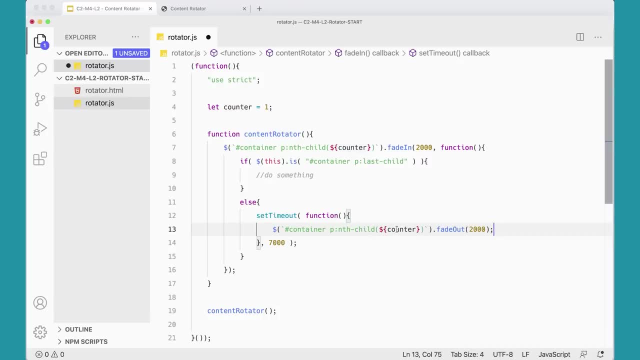 If it's not, it's going to wait seven seconds. After those seven seconds are over, it's going to fade that thing out over two seconds. When it's done fading out, we need another callback function. So I'm going to stick another function in here. 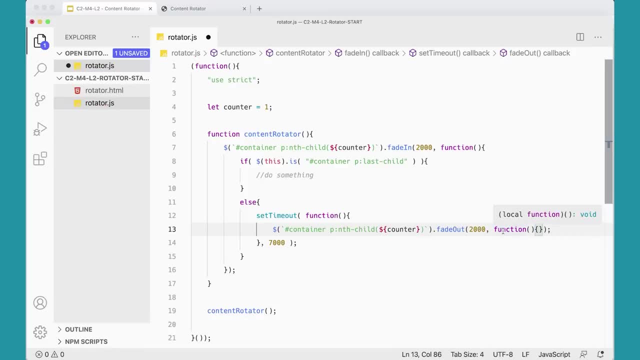 Like so. So it gets confusing, Because now we have a callback inside of a callback. Now, sometimes this is referred to as callback hell, But this is the way we need to kind of get this thing to work well, And we actually have a callback inside of a callback inside of a callback. 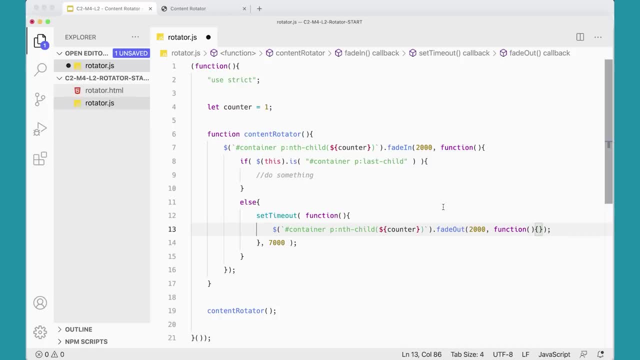 We're doing all of these layers of callbacks here Because we're fading in, we're waiting seven seconds, we're fading out, we're doing three things, So we need to sort of let those three things go. Let those three things stack up there. 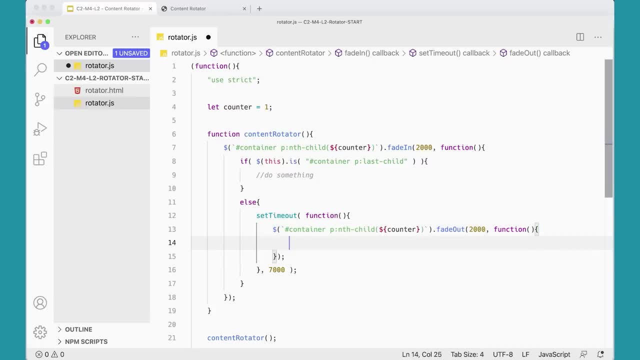 Now in here, what we're going to do is increment the counter, counter plus plus, and run content rotator again. So content rotator runs itself with the counter set to two. It'll check to see if it's the last child. 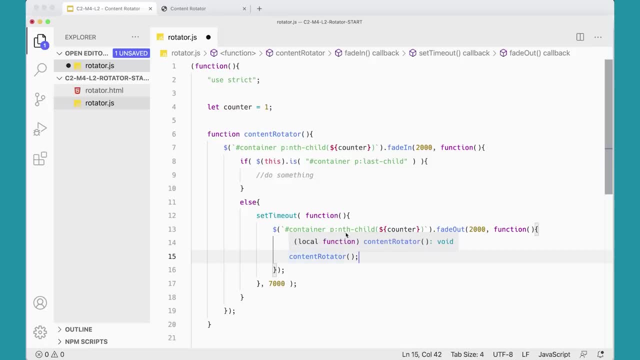 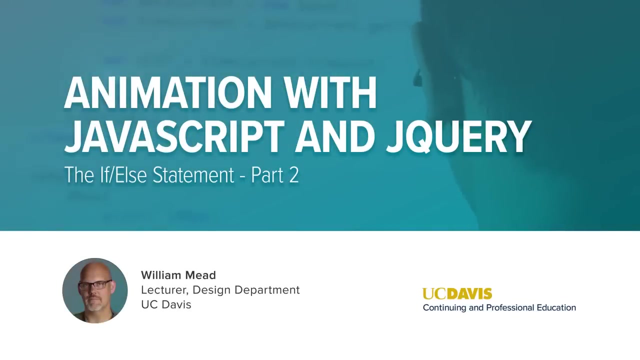 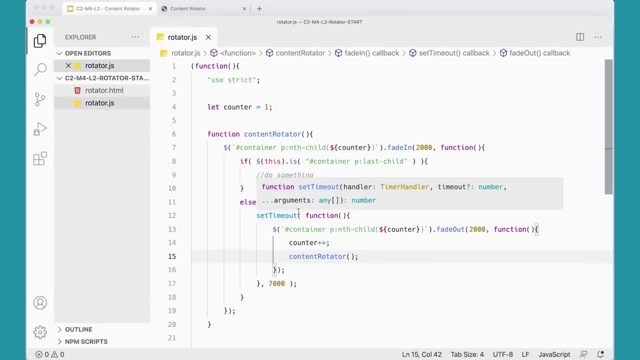 If it's not, it'll do this, It'll increment the counter and it'll do it again And it'll keep going around. All right, great, We'll finish out this part up here in the next video. Okay, in the last video we set our set timeout to wait seven seconds and then fade out the paragraph that's in there over two seconds. 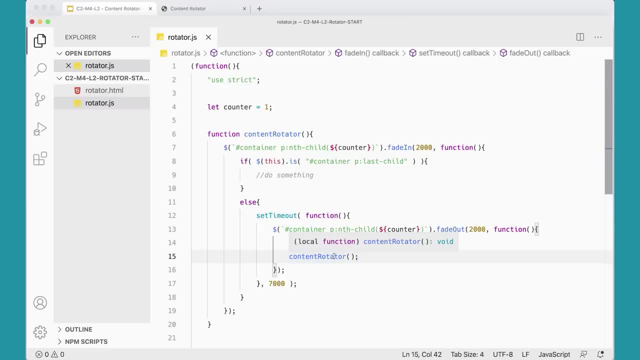 And when that's done, increment the counter and run content rotator again. Now we just have to hand it over. We have to handle the case of what happens if we're on the last paragraph. If we're on the last paragraph, we want to do pretty much the same thing. 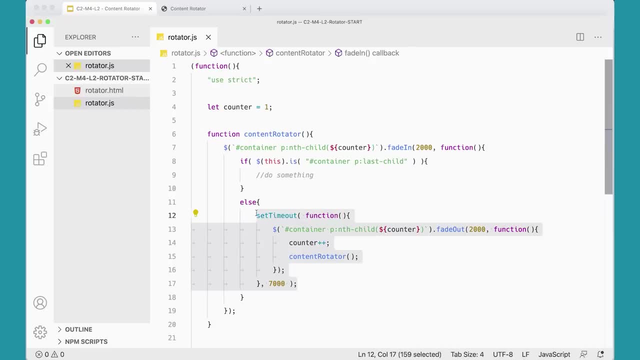 And I could just copy and paste this and stick it in here and make minor changes, But since it's so important to understand this, I'm actually going to type it again. So in here I'm going to add set timeout again. 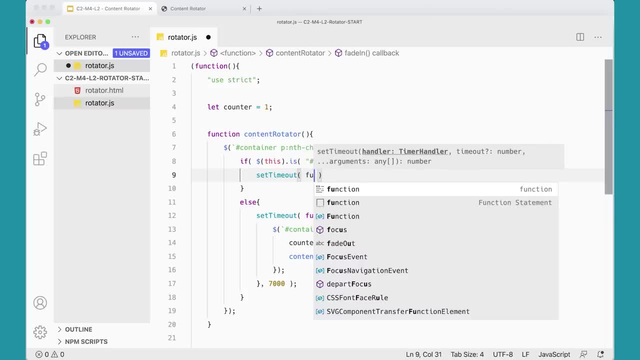 And set timeout runs a function over timeout Over a certain amount of time, in this case seven seconds, like so. So it's going to run this function over seven seconds. It's going to wait seven seconds before it does this function. 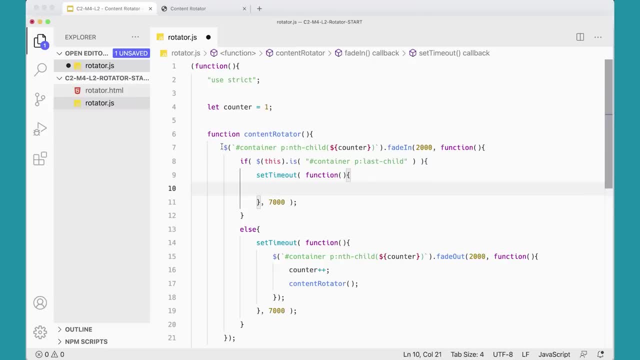 So in here in this part, I will copy and paste, just to make sure I get it right, Just this piece here I'm going to say, okay, go into my container and get that p? nth child counter, which in this case it's the last one. 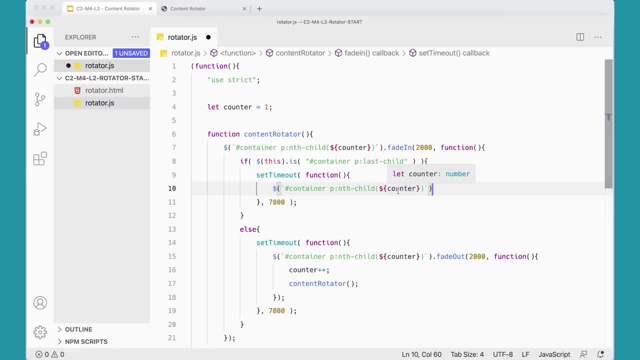 In this case it should be the last one. It should be counter, It should be four, Right, If it's our last child on our thing with four paragraphs in here, So get that one, And then I'm going to do fade out over two seconds 2000.. 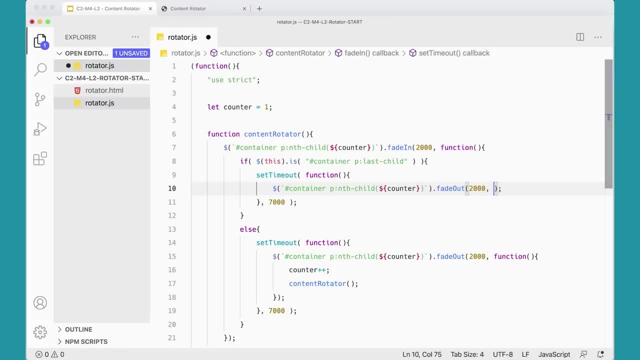 When those two seconds are over, I'm going to run another callback function. Okay, Again, I have to wait until those two seconds are over before I can do this, And here the one thing that's different from what I did below is the counter gets set to. 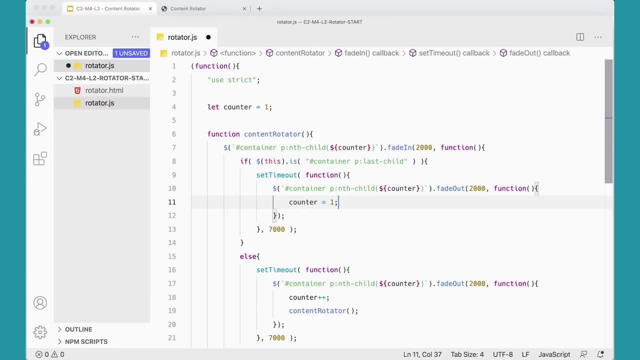 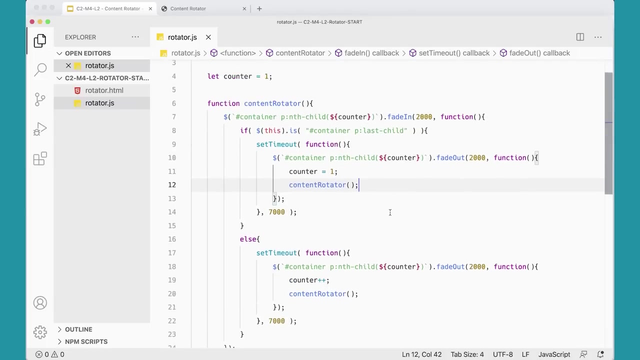 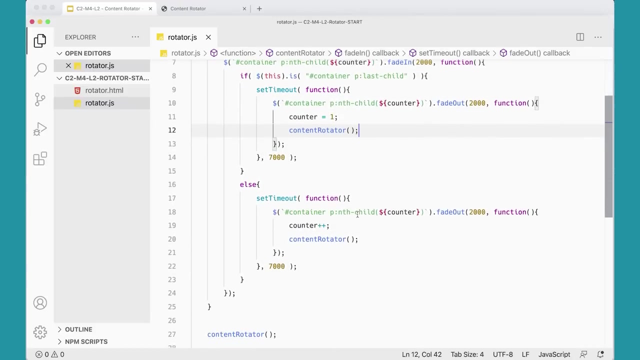 one. So I'm setting it back to my first paragraph and then I'll run content rotator again. and now content rotator will run Another time, But now with the paragraph set to one. so that should all work if we did all this right. 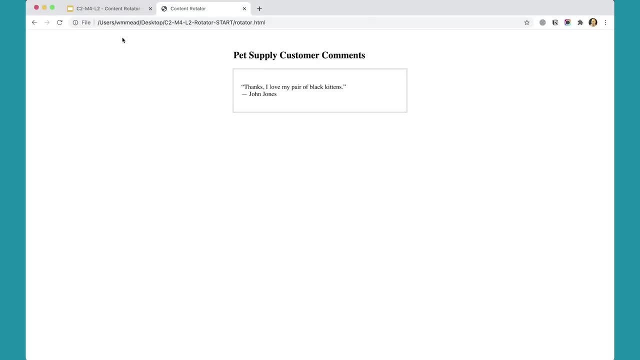 So let's go over and test it out. If I come back to my page over here and click refresh, You can see that it's fades in the first paragraph over two seconds. Then it's going to wait for seven seconds because you know it takes you seven seconds. 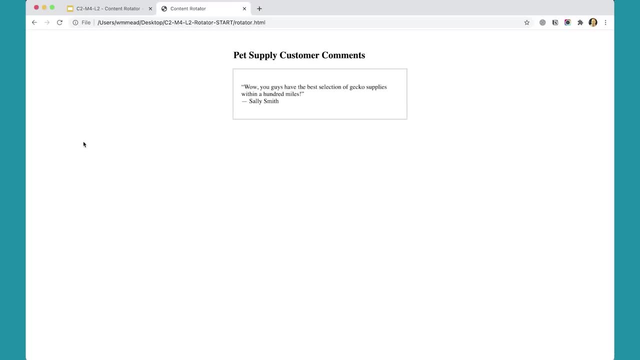 to read that sentence and then it'll fade it out and fade in the next one. That one's on the screen for seven seconds. If you wanted to test this a little bit faster, you can change the seven thousands to say three thousands or something like that, and it would run a little bit faster. just to test. 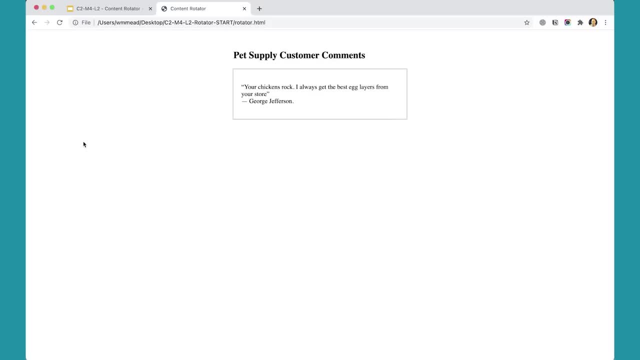 it, But I really want to let it sit there for seven seconds. I think that's enough time to read. And then it comes back to the first one and it's going back around and around and around, and this will just continue forever. In summary, hopefully through this project, you saw that you can use callback functions. 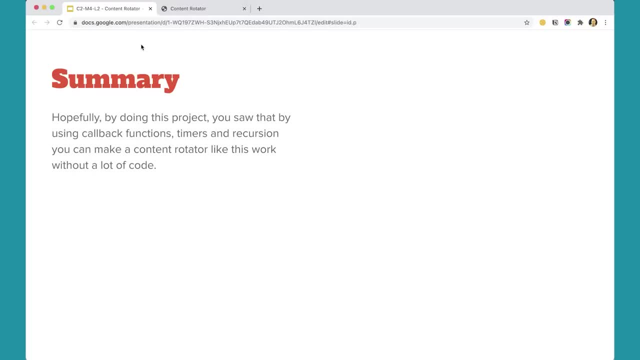 timers and recursions, to make something like this content rotator work without a tremendous amount of code, especially in combination with jQuery and the built-in effects library, Although it would be interesting to make the same script work without jQuery. That would be a good challenge for you. 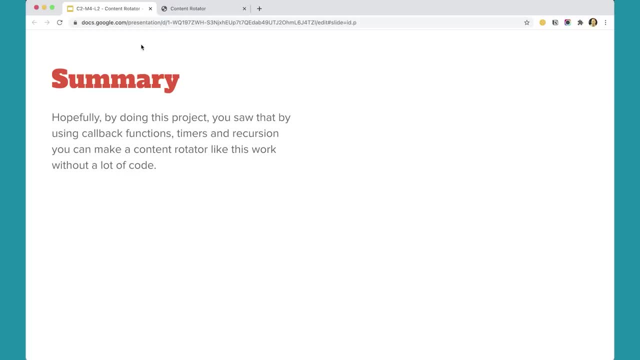 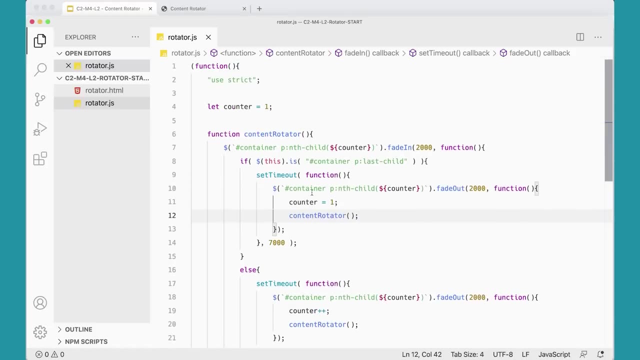 See if you can do that, Or what else could you make work with this script? The script is fading content in and out, And we're right now we're fading in and out paragraphs on our HTML here. but it really could be anything. 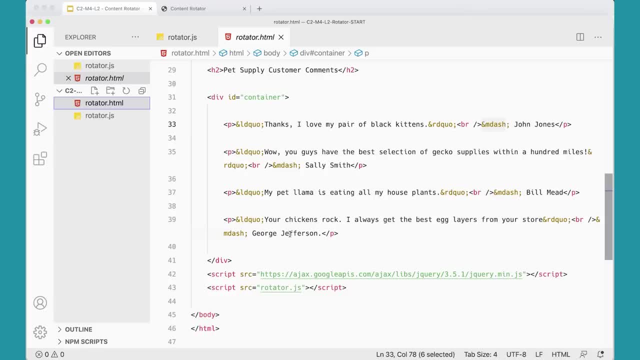 And I could add paragraphs. That's another thing Is that If I were to handle an unlimited number of paragraphs, I could just keep adding paragraphs in here and the script will just work. So that's kind of nice, But what if it wasn't paragraphs? 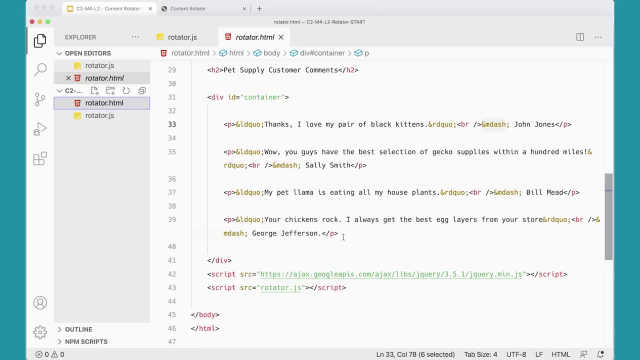 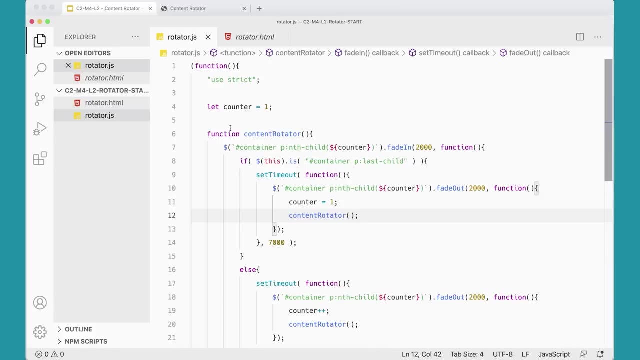 What if it was pictures or block quotes or other types of content that got rotated in and out? You could rotate anything and see how that you know, see how you would need to modify the script to make that work. Other things that are exciting about: about recursion in general, or, yeah, the way recursion. 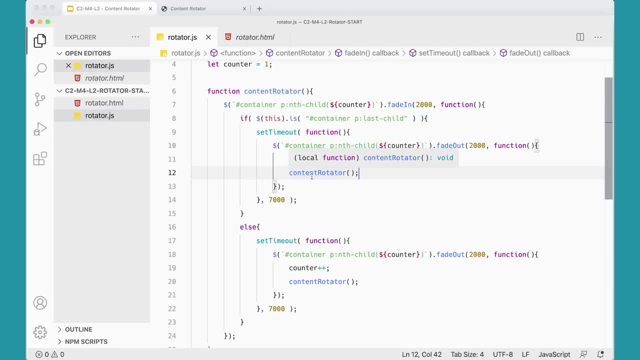 works is that you could make a recursive function that takes parameters and you could run that recursive function passing in different parameters each time it runs. So that makes recursion very interesting and very different than just a simple loop, because you could run the same program but the program could do something different each time. that 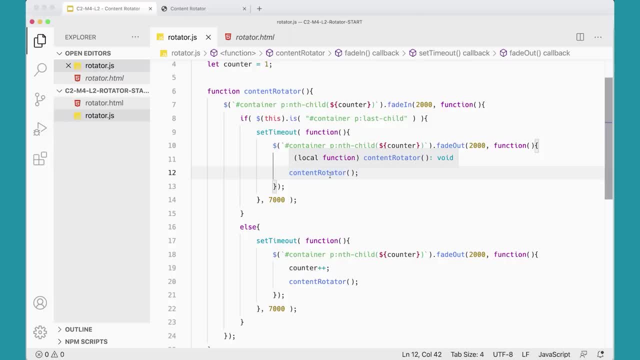 it runs, And that's very interesting to think about. Think about what you could do with that. There's a lot of really fun projects you could make where using recursion, where after a certain amount of time, the function runs itself again, but with a different set of parameters. 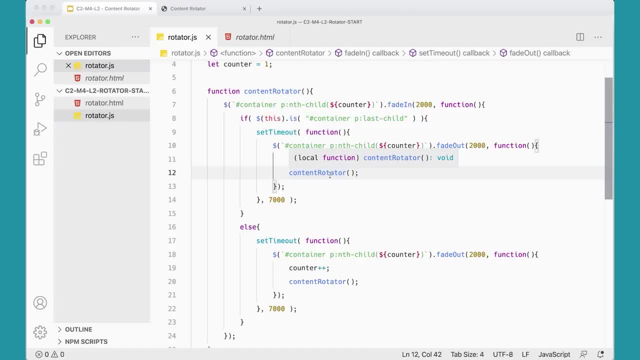 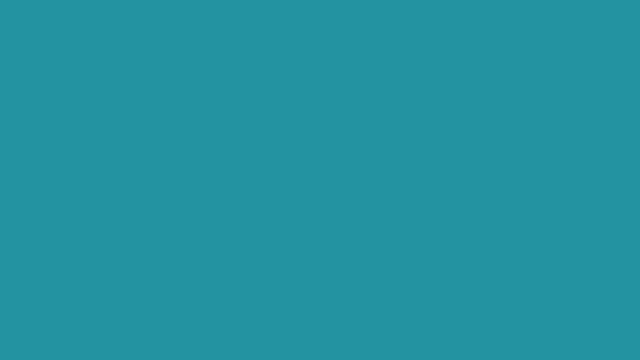 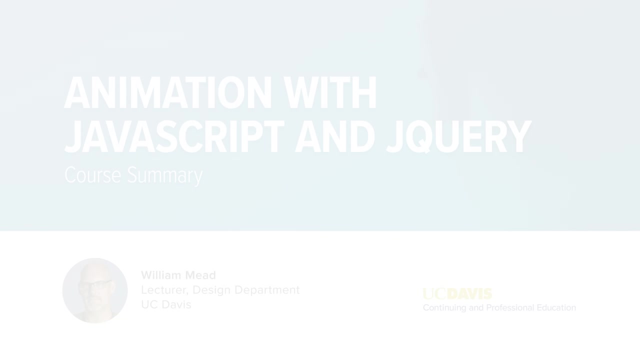 You could even use the random function to pass in random parameters so that you don't know what you're going to get each time the function runs itself. That can be very interesting. Congratulations for making it to the end of our second course on JavaScript in our 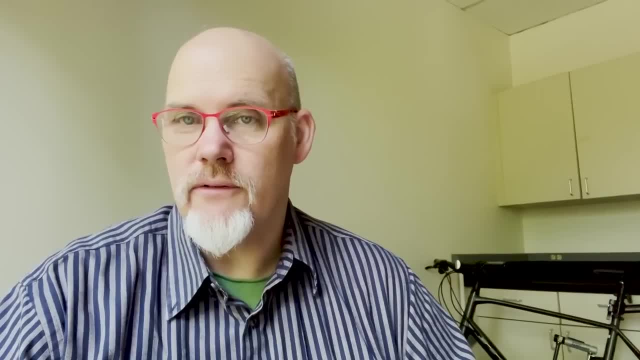 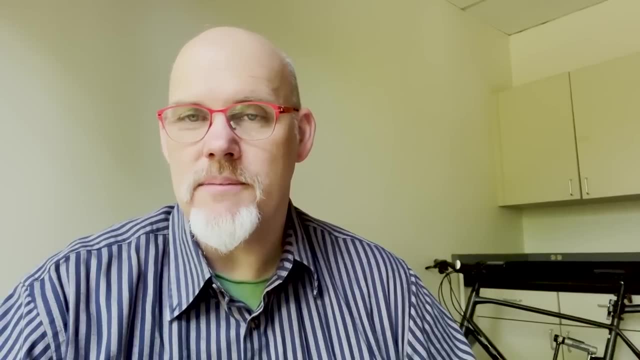 four course specialization. You've learned a lot of JavaScript so far, as well as tackling jQuery and jQuery animation and animation using CSS and JavaScript. We've created some fun interactive elements you can put on real websites. I think you've learned a lot. 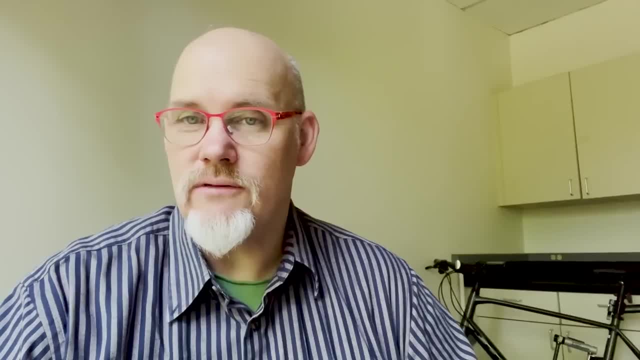 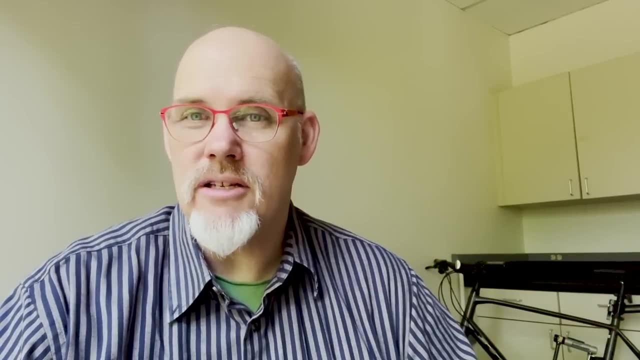 And you should be really proud of yourself. So congratulations for making it this far, And I look forward to seeing you in our third course on JavaScript, where we'll get even deeper into the jQuery library, jQuery plugins. we'll create some more sophisticated scripts. 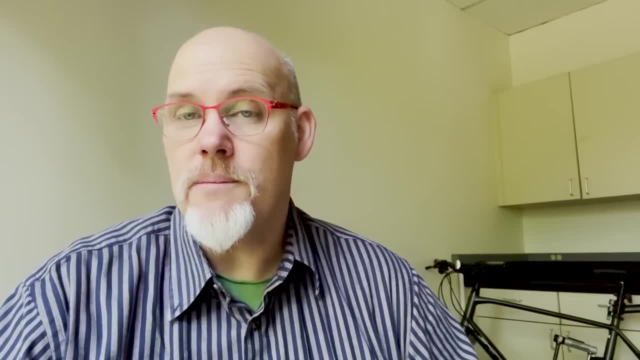 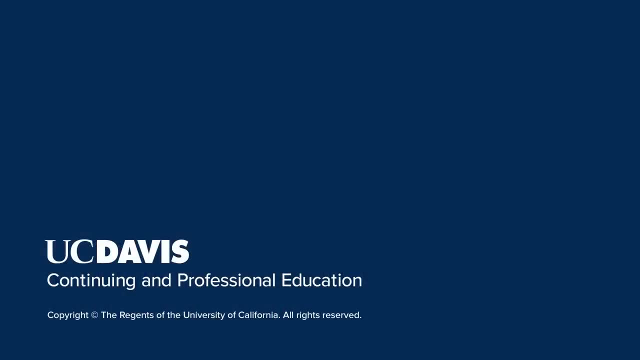 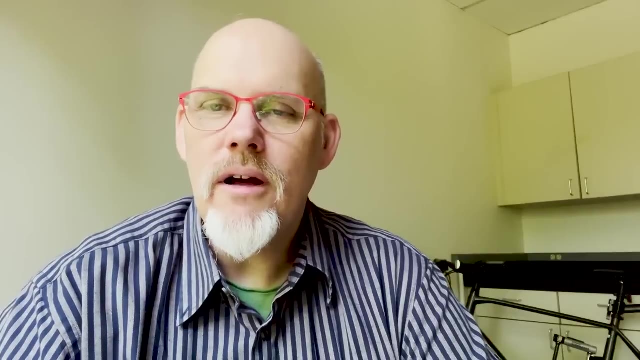 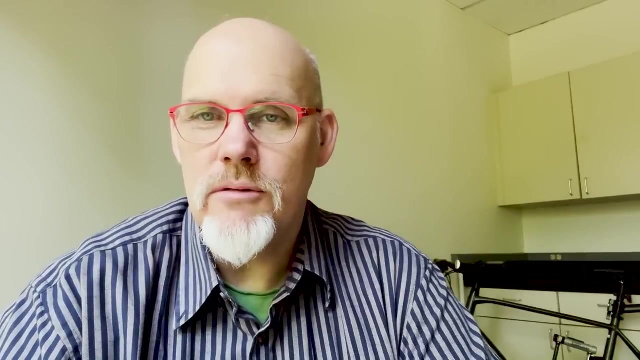 and some more complex scripts so that you can really develop your skills and get better at JavaScript. So I look forward to seeing you there. Hello and welcome to our third course in our four course specialization on JavaScript. My name is Bill Mead and I'm back again to do more JavaScript with you. 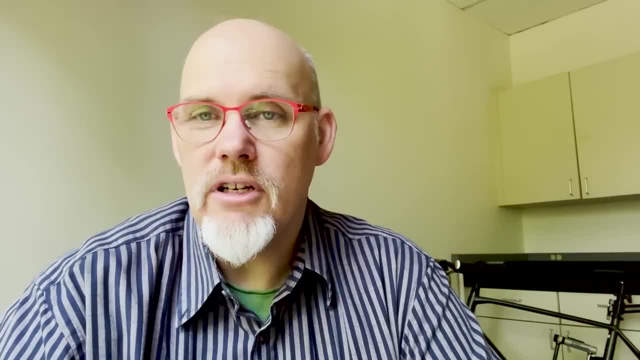 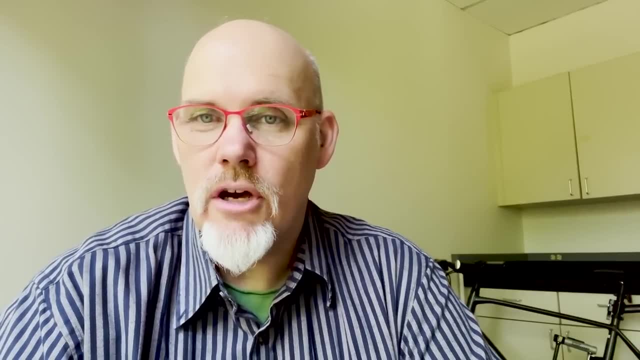 Hopefully you've completed our first two courses on JavaScript and you've learned a lot about the syntax of JavaScript and how to solve problems with JavaScript. It takes a lot of practice to get good at this stuff. So I'm back again to do more with you, to introduce some new concepts, to do some new projects. 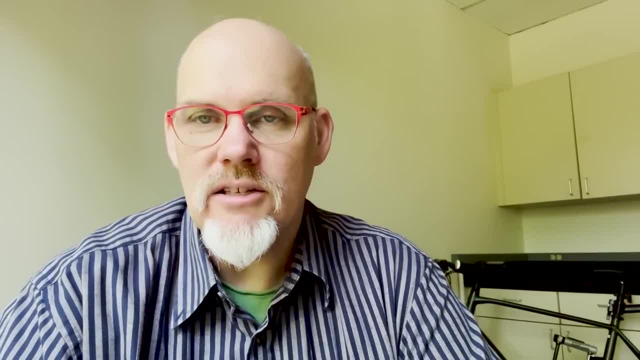 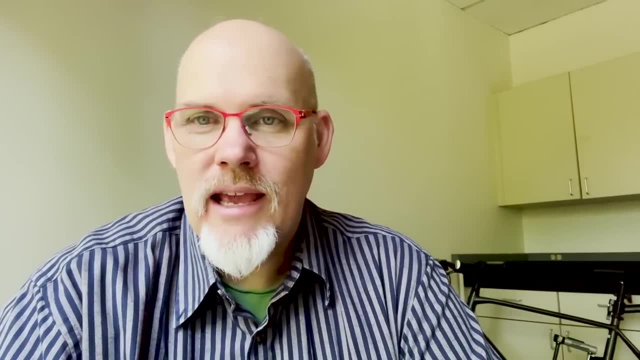 and to do some more sophisticated projects And give you even more practice So you get even better with JavaScript and jQuery. We're going to do a lot in this course, So let's break out our code editors and our web browsers and get started and learn even. 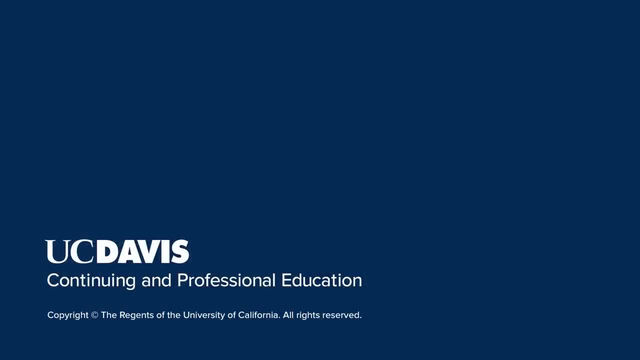 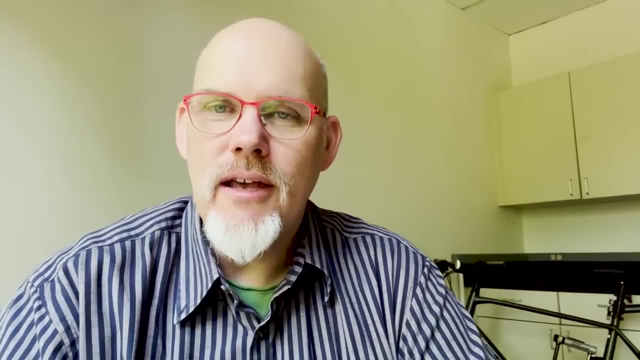 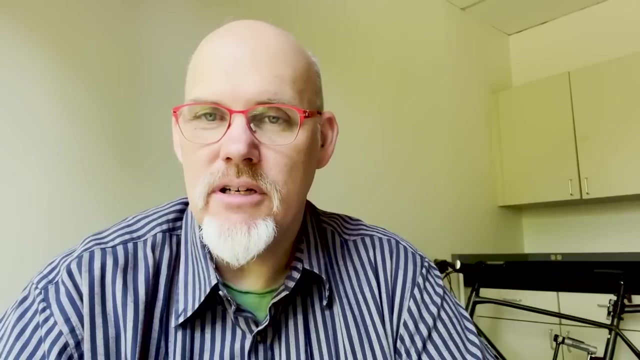 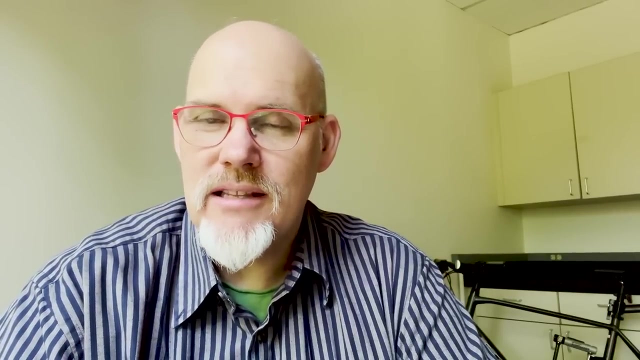 more about JavaScript. Hello and welcome to our first module in our third course on JavaScript. In this module, we're going to dive even deeper into JavaScript and we're going to dive even deeper into jQuery, looking at some jQuery plugins. You've already made some sliders in a previous lesson, but in this lesson we'll look at 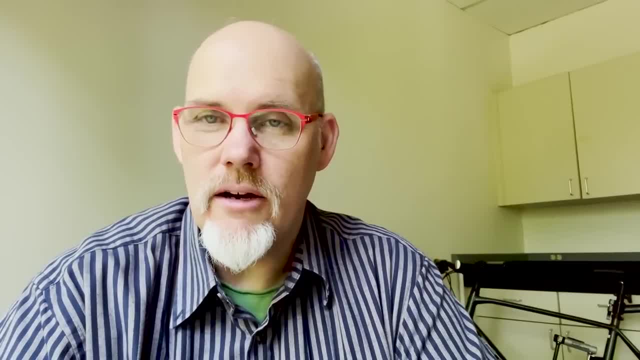 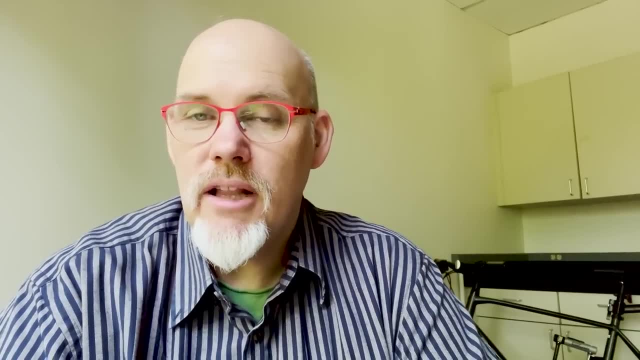 the Flex Slider plugin, which adds a lot of features to sliders, And comparing that to what you've done manually by creating your own sliders is really instructive and useful. Plus, you end up with a great tool for creating slider elements on web pages, and that's really. 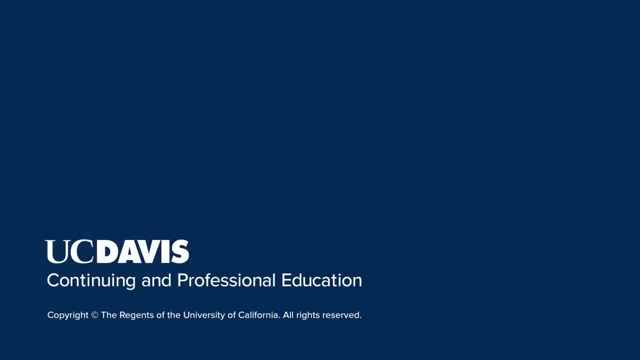 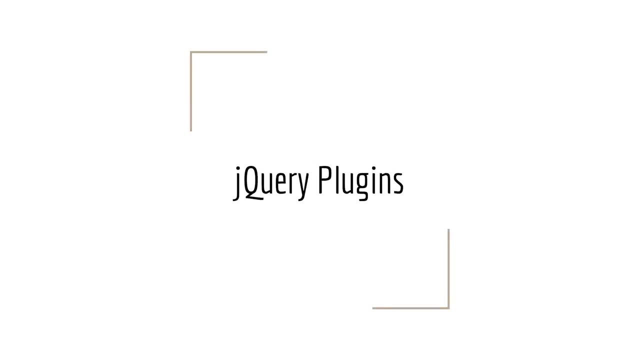 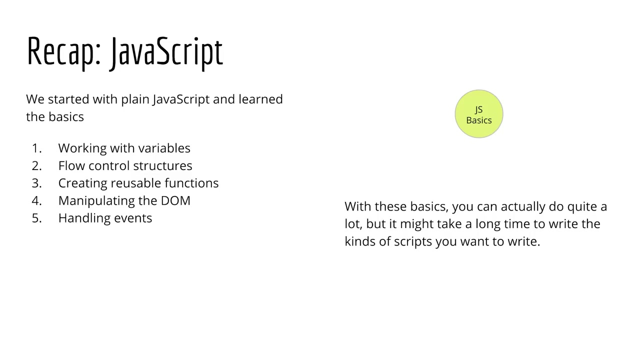 pretty fun JQuery plugins. Just as a quick recap, we've learned a lot of JavaScript so far. We started with the JavaScript basics, which included working with variables, flow control structures like if statements and else statements and loops and that kind of stuff. 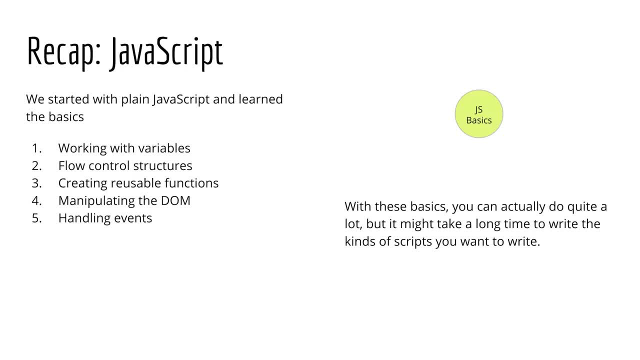 We created reusable functions that you can use in multiple projects or you can use multiple times, And we've done that in the same project. We've manipulated the DOM and handled events such as when somebody clicks on something or hovers a mouse over something. 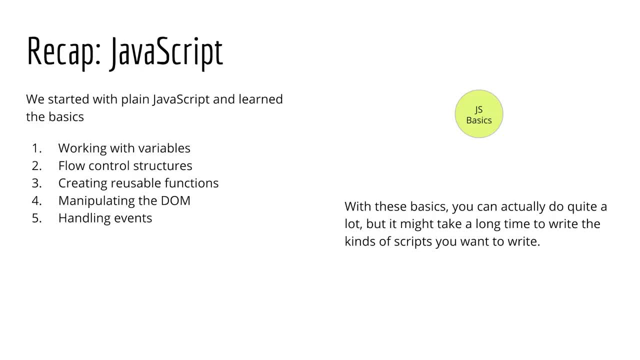 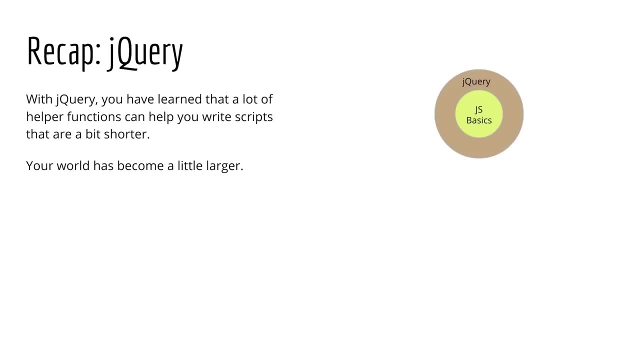 We can capture those events and then do things with them, And with these basics you can do quite a lot, but it might take you a long time to write the kinds of scripts that you want to do for your web page. Then we added jQuery and your world became a little bit larger. 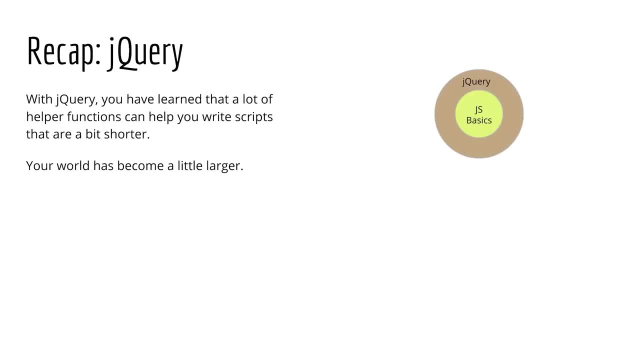 With jQuery, We've learned that there are a lot of helper functions built into this library that make writing scripts shorter and a little bit more compact and a little bit easier. So that helps and that makes things a little bit easier and a little bit better for all. 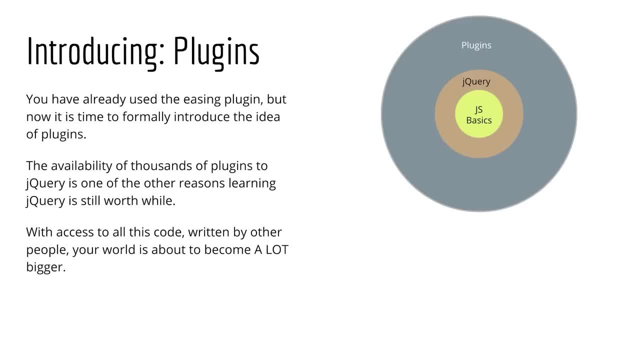 of us. Now we need to introduce plugins, and we've already used the Easing plugin, which is a very simple plugin that adds additional function to jQuery That allows it, So that you can use it for a lot of different things. We've learned that there are a lot of helper functions built into this library. 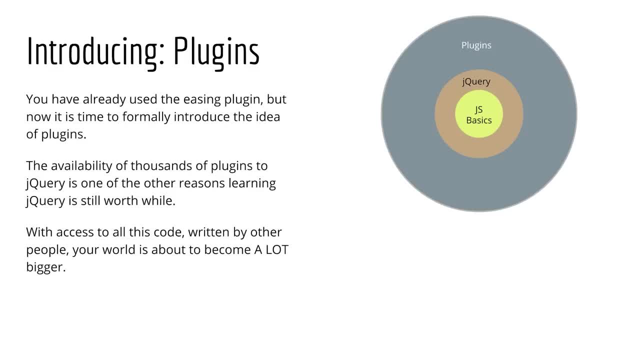 We've learned that you can use different types of Easing, which is different speeds and ways in which things can animate on your screen, And by plugging in that particular plugin, you get access to all of those different features that aren't built into jQuery. 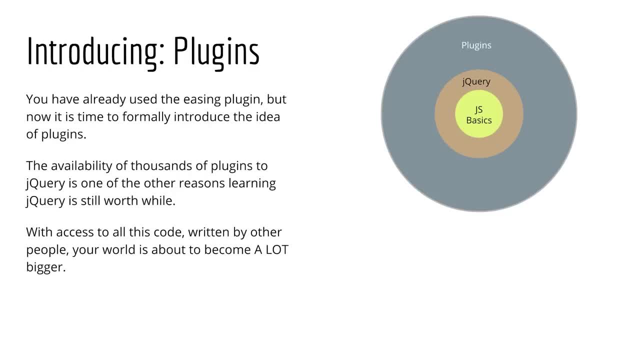 And jQuery has this plugin architecture that's very powerful, that allows developers to build extensions to jQuery that give it a lot of additional functionality, And there are Tons Of JQuery plugins available- thousands of them- And I recommend looking around the web and seeing what other ones you can find. 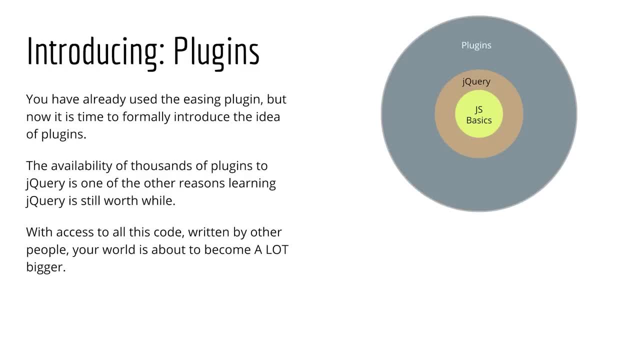 We will look at one or two here in this course, but there are just thousands of them out there and they're really worth exploring and seeing what's what's out there, And so that way your world becomes a lot bigger, because now you don't only have to. 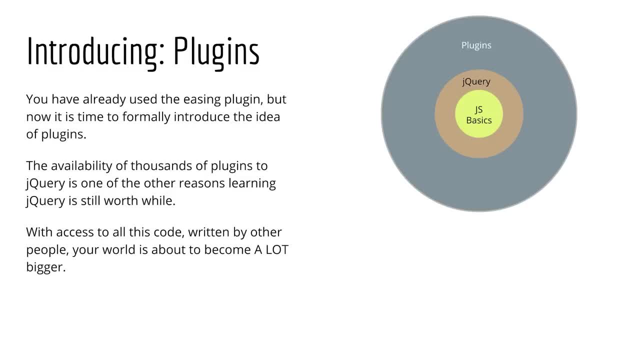 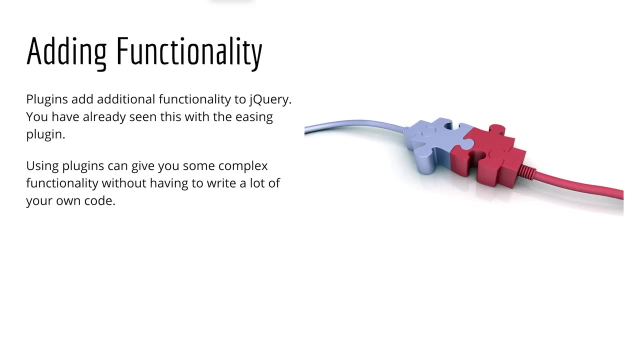 Just write all your scripts yourself. You can look for scripts that other people have written and see if you can modify them and use them in your own projects through the use of a plugin, And that's really very powerful and really great. Again, plugins add additional functionality to jQuery, and we've already seen this with 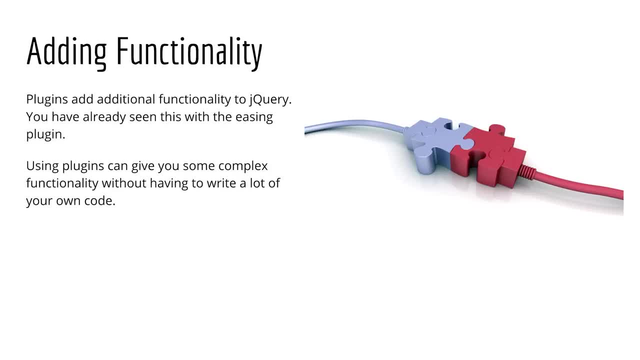 the Easing plugin, but some plugins can have very complex functionality. Not us having to write a whole bunch of code. We have access to a whole bunch of additional functions and we'll see what that looks like. You can create whole interfaces in a jQuery plugin and then, by providing that plugin, 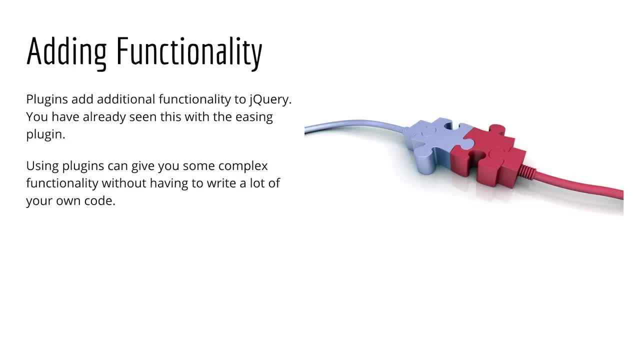 other people can have access to those interfaces. So, for example, we did the project where we made the tabbed interface. What if there was a jQuery plugin that made hooking up a tabbed interface super easy? And there are plugins for that. 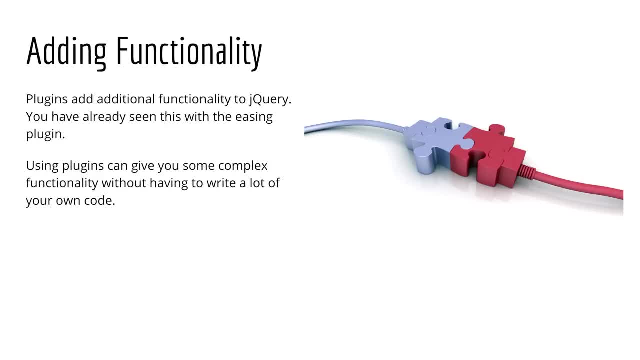 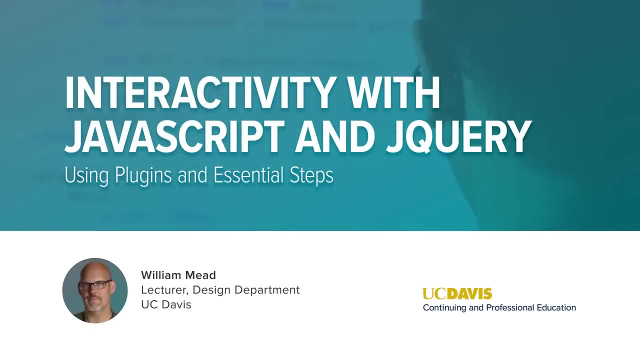 For those kinds of things, And they might come with a lot of features and functionality. What if you want the tabs to run down the side of the tabbed interface rather than across the top? You could do that kind of thing Using plugins and essential steps. 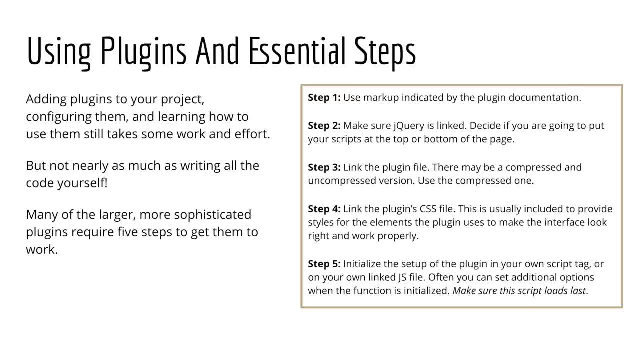 Adding plugins to your project, configuring them and learning how to use them still takes work, some work and effort, but not nearly as much work and effort as it takes to write the whole script yourself. Many of the larger, more sophisticated plugins require five steps to get them to work. 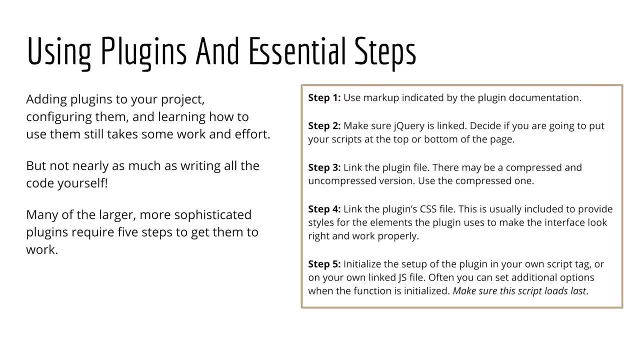 Step one is you have to use the markup indicated by the plugin documentation. Often, you'll have to use divs or articles or other elements with particular classes that the plugin needs in order for it to actually work. Classes or IDs or other structures that the plugin needs for it to work. 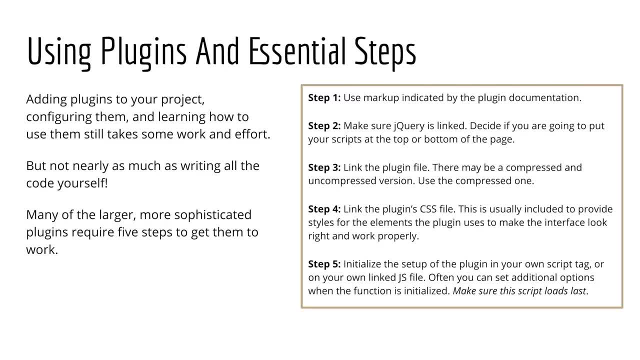 And then you need to make sure jQuery is linked, the jQuery library is linked, Because if you're using a jQuery plugin, then you need to have jQuery. Decide if you're going to put your scripts at the top of the page or at the bottom of. 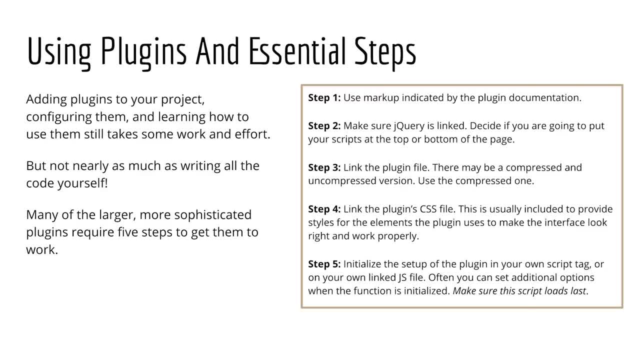 the page. Sometimes you can put them whichever place you want. Sometimes the plugin directions will tell you to put them in one place or the other, But frequently it might need to be in one or the other place depending on your spatial. But frequently you can make your own decision on this and put it where you want it to go and architect your file the way you want it to be structured. 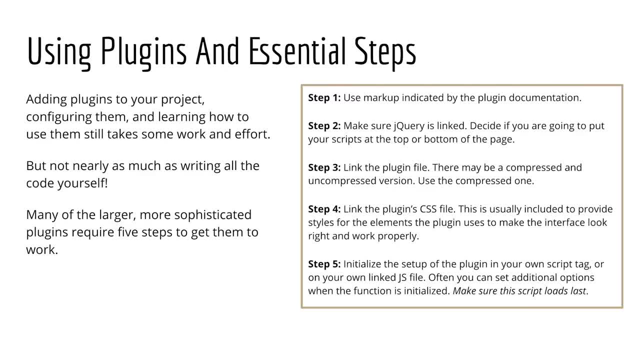 Step three is to link the plug-in file, And when you download a plug-in, frequently it will come with a compressed version and an uncompressed version. The uncompressed version is there for you to look at so you can see how the plug-in actually functions. 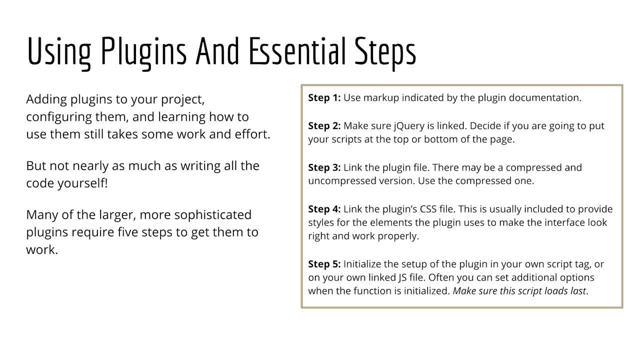 It's readable JavaScript and you can do that kind of thing. But when you're ready to put it into your project and for your production-ready project, you want to use the compressed version because it'll be smaller and it'll download faster. So if they provide a compressed one, then you should use that. 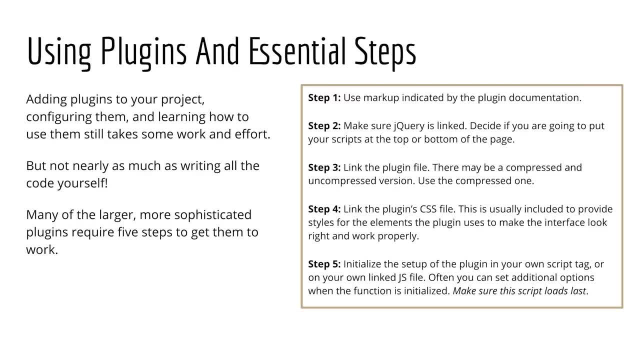 If they don't provide a compressed one, you can compress it yourself. Step four: link to the plug-in CSS file. Some of the fancier plug-ins will come with styling that will style the elements inside of the plug-in, And this is usually included so that everything looks and works the way it's supposed to work within the interface for that plug-in. 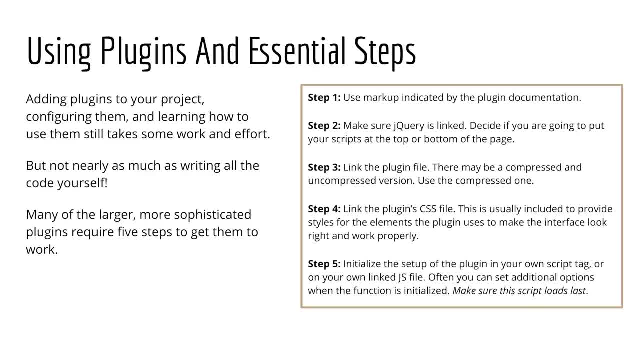 So you want to make sure you get that CSS file linked onto your page. Then step five is you need to initialize the setup of the plug-in in your own script tag or on your own linked JavaScript file. Often you can set additional options So that when the function is done, you can set additional options. 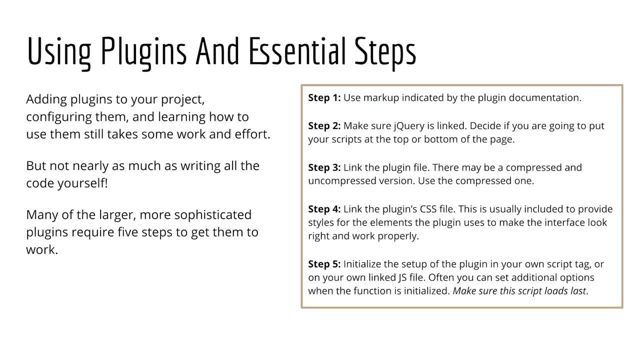 So that when the function is initialized and so that you can pass in whichever options will get the plug-in to display the way you want it to display. But you want to make sure that this script loads last. So the order of things are that you will have the jQuery plug-in, then you'll have jQuery, then the jQuery plug-in and then you will initialize the plug-in on your own script. 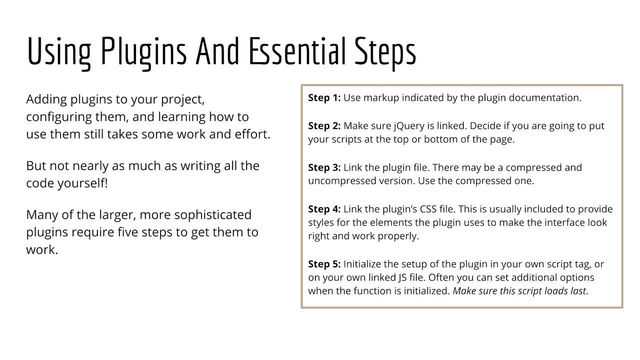 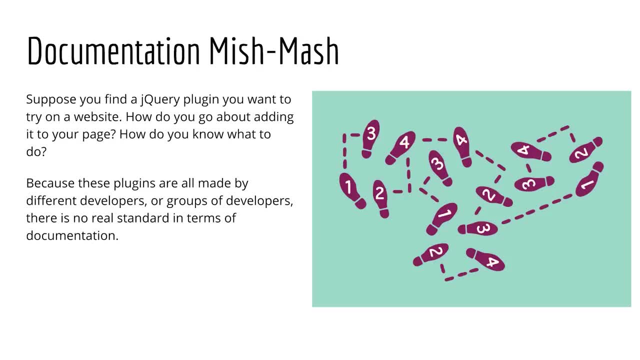 And then also make sure that if there's any CSS files, those are included as well. Documentation mishmash. Suppose you find a jQuery plug-in you want to try on your website. How do you go about adding it to your page? How do you know what to do? 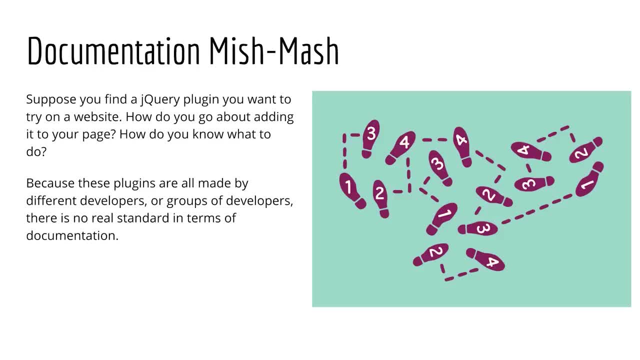 Because these plug-ins are all made by different developers or groups of developers. there's no real standard in terms of the documentation. So this is where having a solid foundation in JavaScript really helps, Because you need to look at the documentation they provide and be able to tease it out and go. 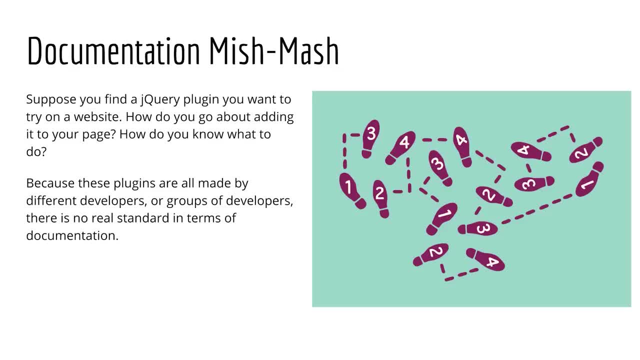 okay, I understand what they're asking me to do here On this page. they're telling me to install the plug-in like this and then add these configuration options and so on and so forth, And unless you have some experience with JavaScript, it's going to look like a bunch of messy code and it's not going to make a lot of sense. 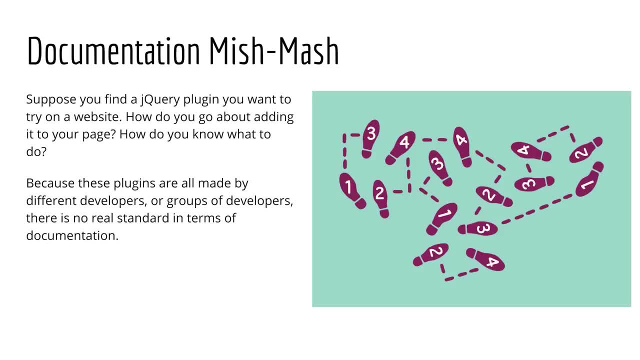 So that's why it's really helpful to have a solid JavaScript foundation before trying to mess around with this stuff. But now that you do, And you'll see once you work with a few plug-ins, that many of them work pretty much the same way. 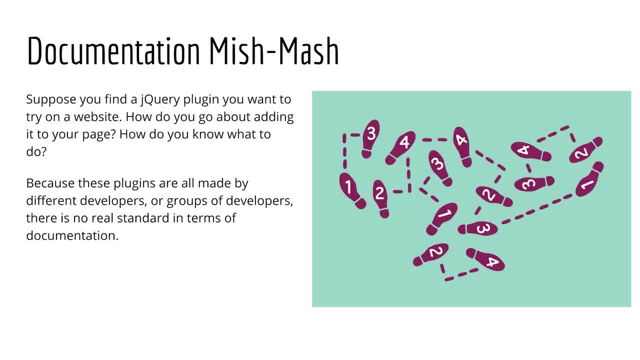 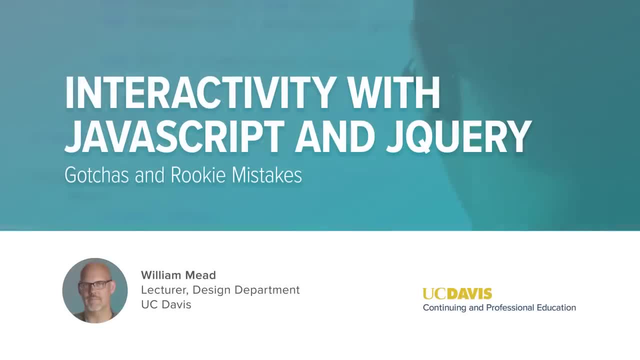 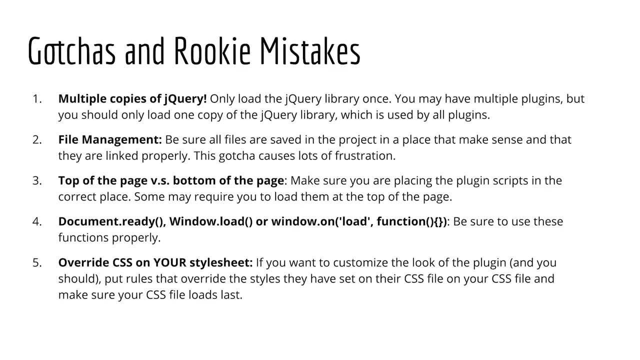 The documentation may look a little bit different, The directions may be written a little bit different, but it's the same basic steps each time: Gotchas and rookie mistakes. Number one on this list is the biggest one. I see this all the time. 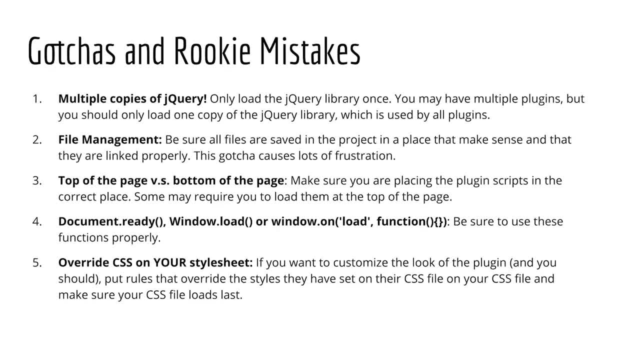 Especially with students who are new to working with JavaScript and jQuery, And that is ending up with multiple copies of the jQuery library linked to your page. Only load the jQuery library once. You may have multiple plug-ins, but you should only load one copy of the jQuery library which is used by all the plug-ins. 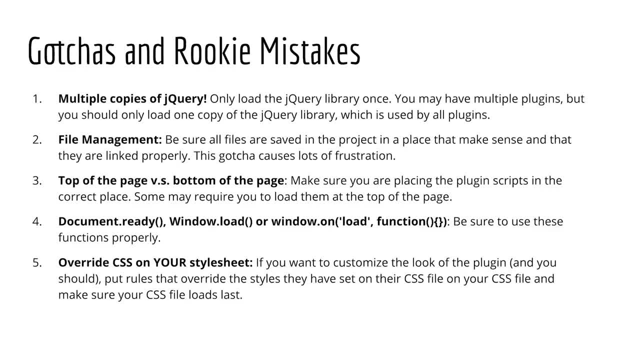 So what happens is you find a plug-in that adds some interesting functionality. You want to use it. So you follow the directions and load the jQuery library and do all the directions to make that plug-in work. Then you find another plug-in that does something else that you want to use. 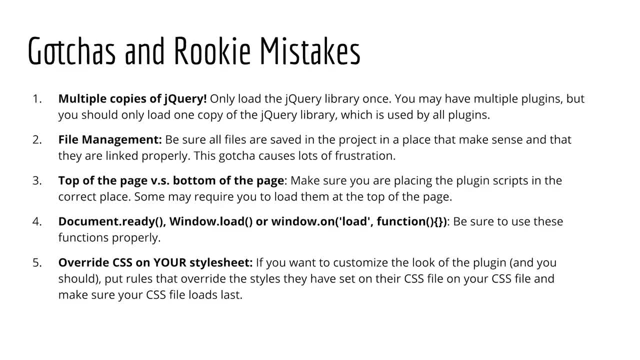 So you follow the directions on that page and it tells you to load the jQuery library and to load the plug-in. So you follow those directions And then in the end you end up with the jQuery library loaded twice And frequently. when you download these plug-ins, they'll include a copy of the jQuery library. 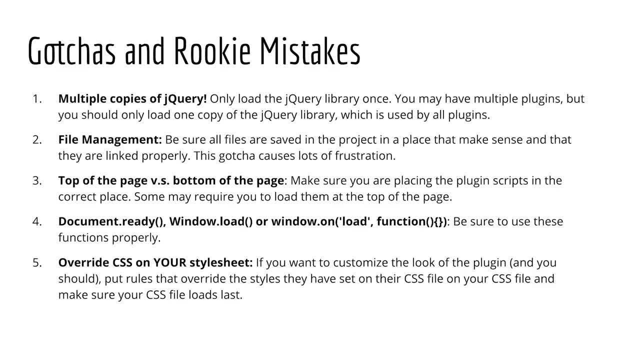 So you'll follow the directions, You'll link up one, then you'll link up another, And it turns out that the two plug-ins you hooked up actually are using different versions of the same jQuery library. So now you've got two different versions of the jQuery library linked up, and that's going to cause all kinds of problems. 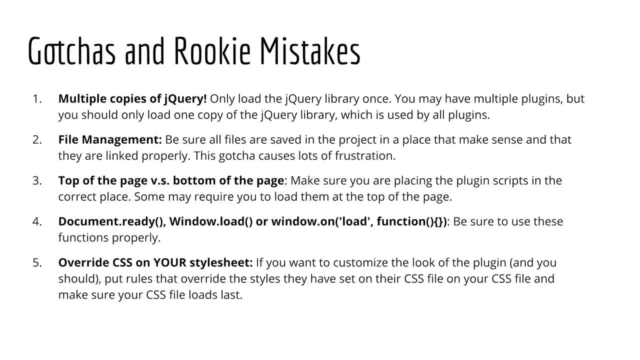 And things will break and it won't work right. So you want to make sure you only ever have one copy of the jQuery library plugged in, And I'm saying this now, but I promise it will happen. I see this. This is the most common error that I see from students who are working with jQuery. 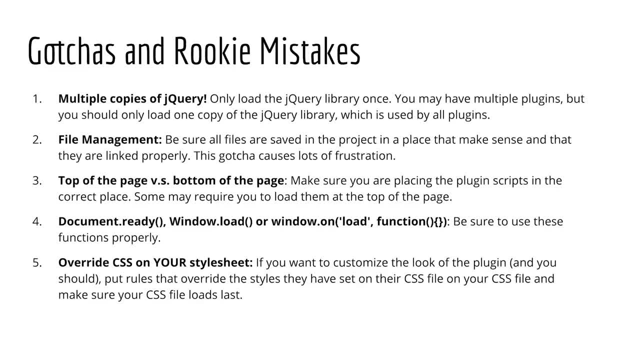 is, they'll follow the directions and then they wind up with multiple copies, different versions of the jQuery library plugged in. So that's the number one gotcha, and it happens. It happens a lot. The second thing is file management. When you download a plug-in, sometimes plug-ins require other files. 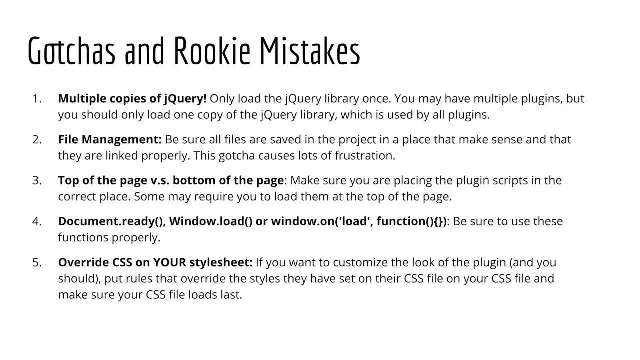 whether it's CSS files or maybe an images folder, Fonts or something else, And you want to make sure that when you put those files in your folder, everything is going into the correct spot and is linked properly, Because for the web, remember, everything is linked. 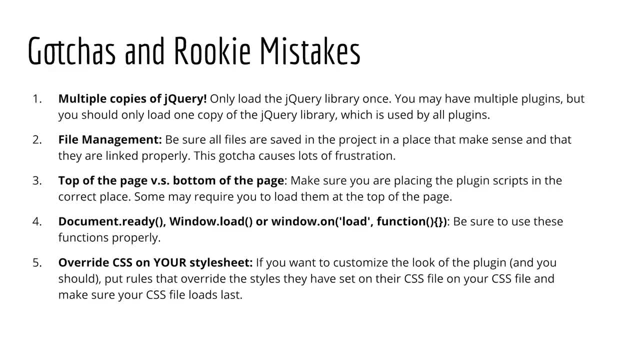 All the files are linked to each other And if those links become broken then your project won't work and it won't work properly. So make sure you have all the correct files in all the correct places for the plug-in to work. 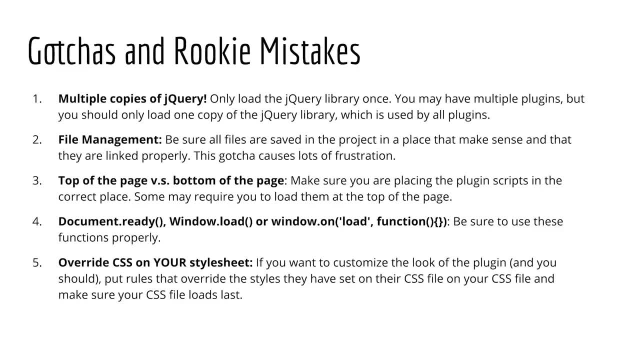 So that's number two. Those two issues comprise 90% of the problems that people have with plug-ins. Probably those two problems. The next thing is top of the page versus bottom of the page. Make sure you're placing your plug-in scripts in the correct place. 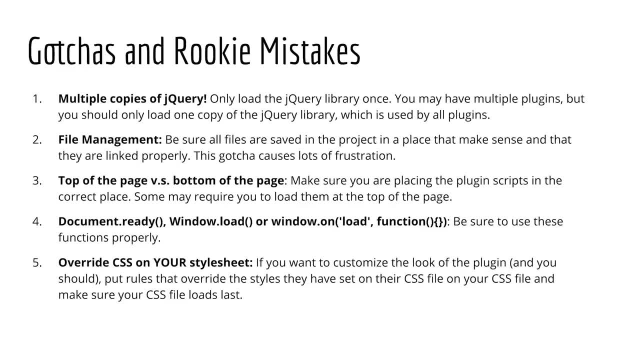 Some of them may require you to load jQuery up at the top of the page. Usually, you can put them Where you want, as long as you run the scripts properly. And that sort of leads us to number four. But make sure you have a strategy for where your JavaScript is going to load. 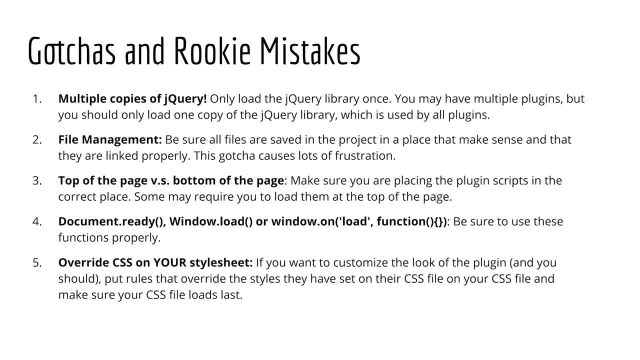 Whether you're going to have it loaded the bottom of the page before the closing body tag, or whether you're going to put the links to scripts up in the top of the page and maybe use the defer attribute to make sure they don't load until the whole page is loaded. 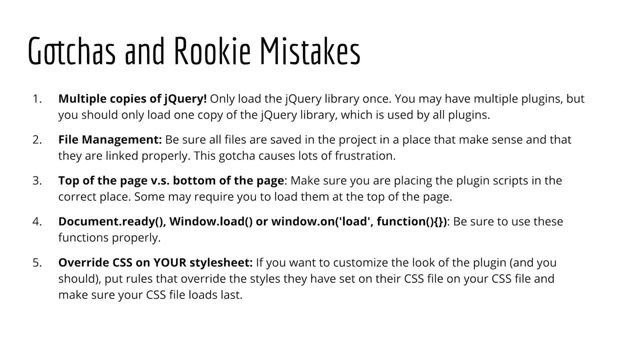 Okay, so keep that in mind. Now, jQuery has a document ready method that will allow you to check and that will check to see that the DOM is loaded. before anything inside the document ready function runs And that's just checking to make sure your HTML is loaded. 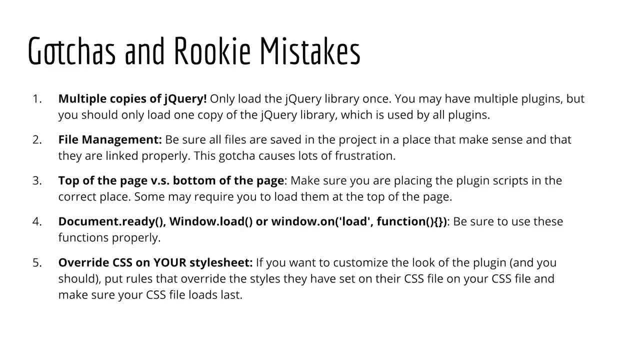 So sometimes people will provide plug-ins and tell you to use the document ready function And you'll need that if you're up at the top of the page and you're not using the defer attribute. But If you put it at the bottom of the page you may not need it. 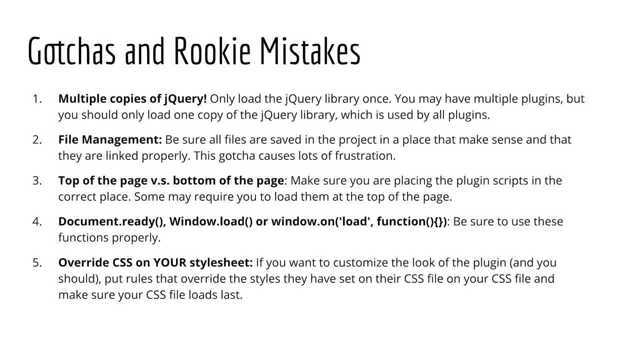 There's also a window load method, And that's in older versions of jQuery, version two and lower. It's now been replaced with windowon And the load And you pass in load as the event that we're looking for and then run an anonymous function. 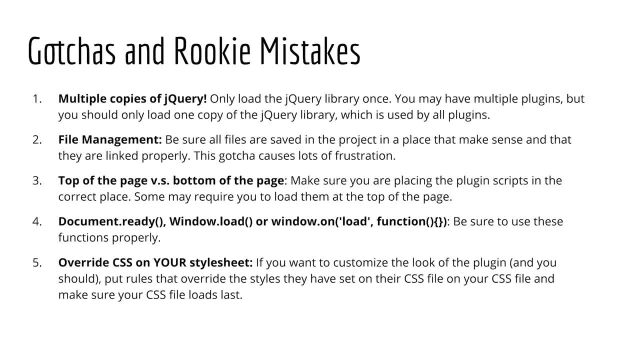 which is what we used in the previous lesson with the sliders. So beware about these different functions, what they do, which versions of jQuery they work with and that kind of stuff, because if you're reading the documentation for a plugin, it could be older documentation. 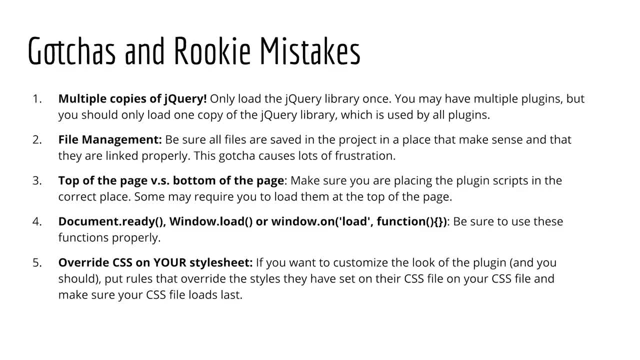 And if you're use, if their documentation is telling you to use windowload, but you're using the most recent version of the jQuery library, you'll have to switch it to the windowon method And And use that, But But. 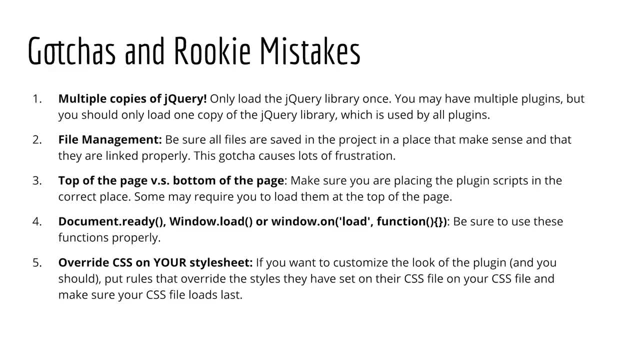 one instead. so you want to make sure that you're using these functions properly and really where you're going to use these is just where you're initializing your script, so it has nothing to do with loading the actual script file or the plugin file. this is where you initialize your script on. 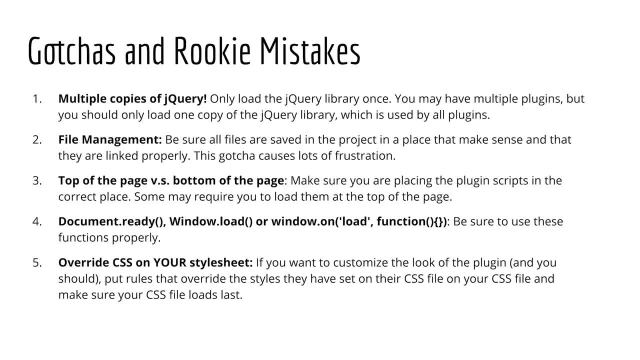 your page where you're telling the the plugin to run. you'll need to make sure you use these functions properly. then number five is overriding css on your style sheet. if you want to customize the look of the plugin and you should put your rules that override the styles they've said on. 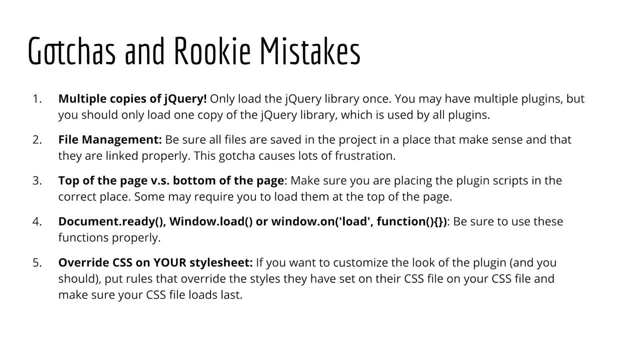 their cs file, css file on your css file and then make sure your css file loads last. that way when you load these up they will um, when yours, when your css loads, it will overwrite the style sheet. override the CSS on their style sheet. You don't want to overwrite the styles on their. 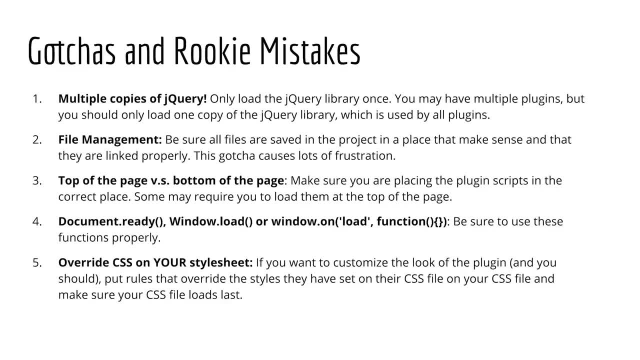 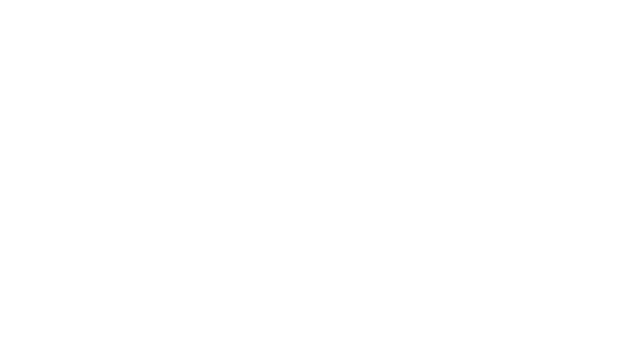 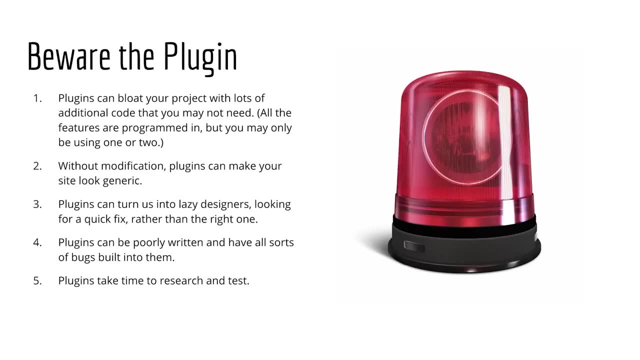 CSS file, because if you ever update the plugin files, you'll lose that and you'll have to do it again. So you want to make sure you put it on your CSS file. Beware the plugin. One last topic that I have to talk about before we're done with this lecture on plugins is just to be aware of the 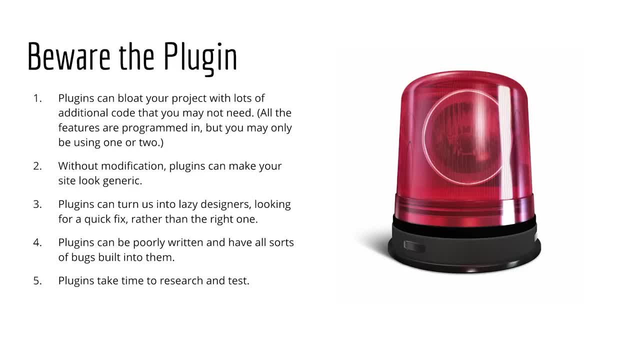 plugin. Plugins can add bloat to your project with a lot of additional code that you may not need All of the features that are programmed into the plugin, but you may be only using one or two, So that's something to be aware of. Without modification, plugins can make your 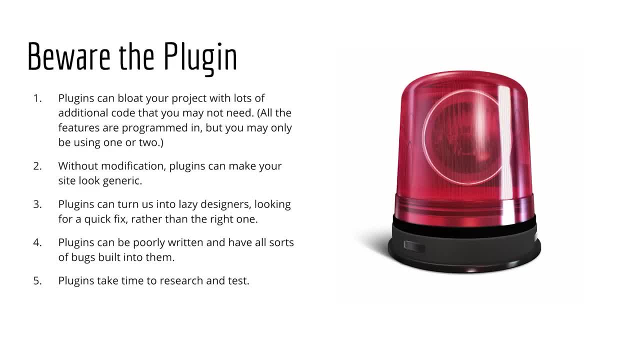 site look generic. So if you're not updating the CSS file or adding your own styles to it, then it could look the same as everybody else's website. Plugins can turn us into lazy designers looking for a quick way to update the CSS file. So if you're not updating the CSS file, then you can. 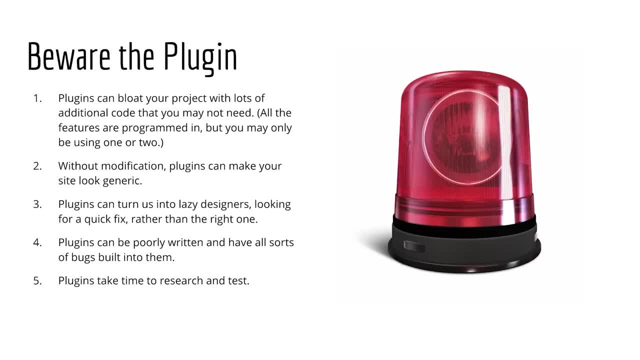 look for a quick fix. So rather than actually trying to solve our interaction design problem, we go look for a plugin that looks cool and interesting. that may not really be the right fit for our project, just to avoid having to do some custom code. So watch out for that. 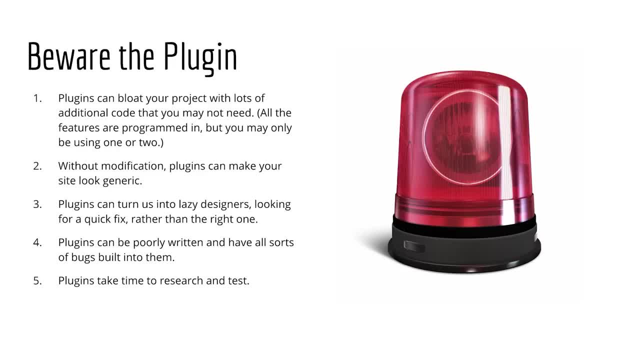 Also, plugins can be poorly written. They can have all sorts of bugs built into them, Because they're made by other developers you don't really know. So you really have to test them out and research them, Find out who else is using them. What kinds of problems have they had? 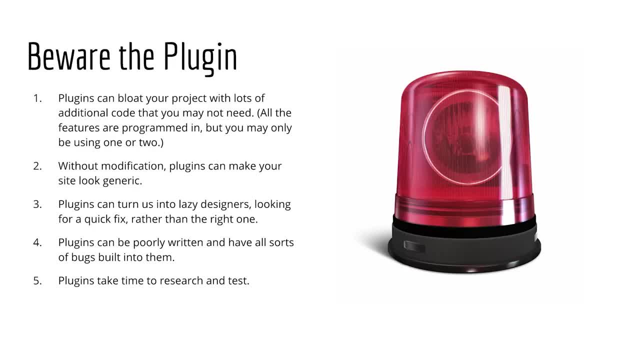 What sorts of things work well with them. It'll take time to do the research, but probably less time than actually writing the code yourself from scratch if it's an extensive plugin, And so it's worth it to make sure that the plugin you're using is really worthwhile. Looking to the future, 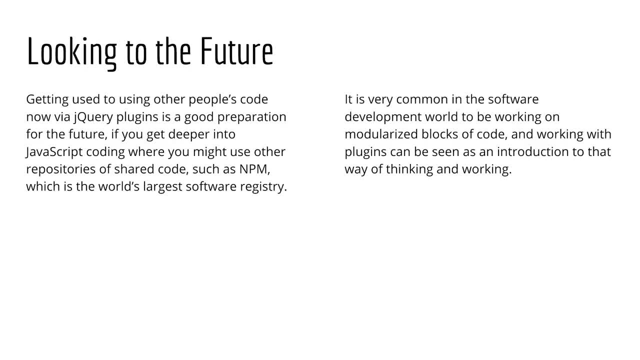 Getting used to using other people's code now via jQuery plugins is a good preparation for the future. If you get deeper into JavaScript coding, where you might use other repositories of shared code, such as NPM, which is the world's largest software registry, then having experience 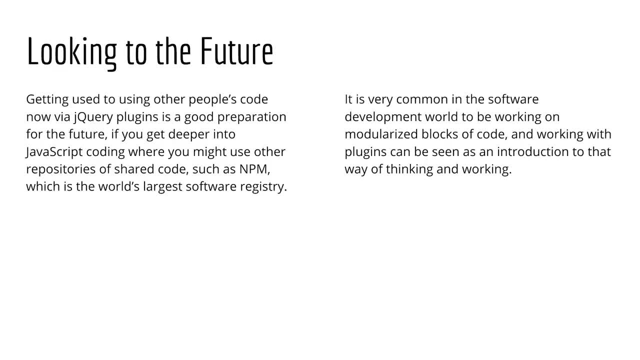 with jQuery and jQuery plugins will really help you out. It's very common in the software development world to be working on modularized blocks of code, And working with plugins can be seen as an introduction to that way of thinking and working, where you're taking sort of 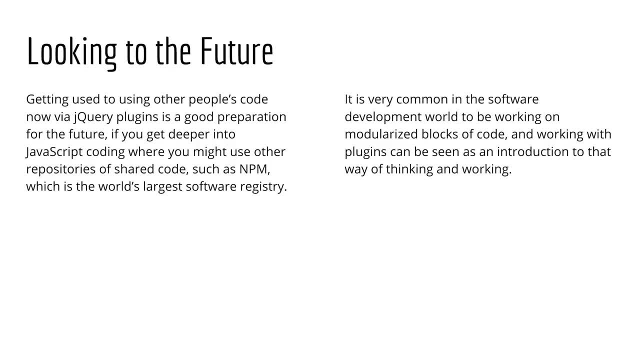 functionality and separating it from the rest of the code. So if you're going to be working on jQuery, you're going to have to separate it out into a separate file and then plugging it in so you have access to that. It's a really great way of thinking and working with JavaScript and jQuery. 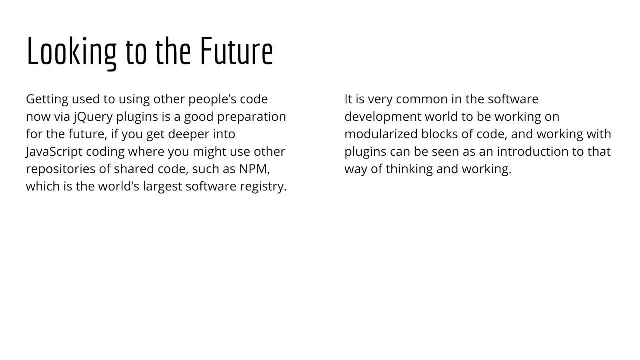 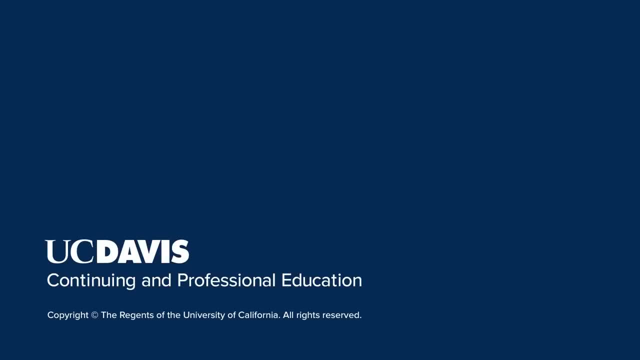 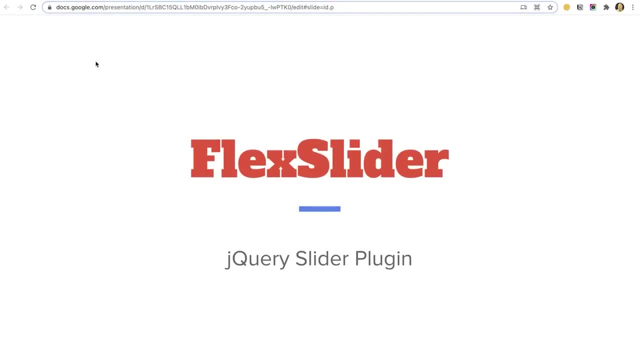 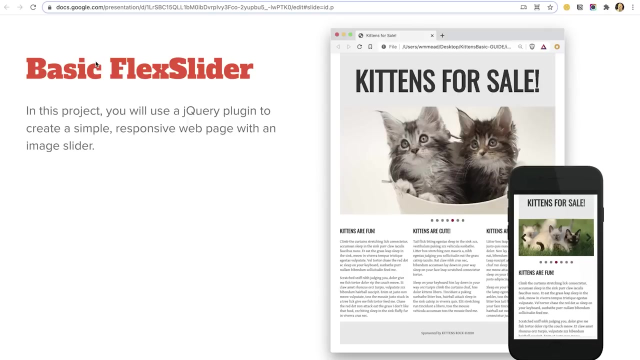 in general, And getting used to that here will help prepare you for a future as a JavaScript developer. Flex Slider- jQuery Slider plugin. Now that we've talked about jQuery plugins a bit, let's take a look at one One that we can use to adds a significant amount of interface options to our page. 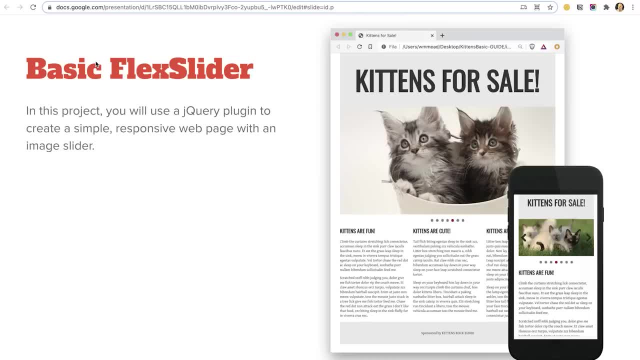 And the Flex Slider is a good one to look at, partially because we've been working on image sliders. So we come to this with the context of having looked at, created some sliders on our own so we can see what this particular plugin has to offer. that's. 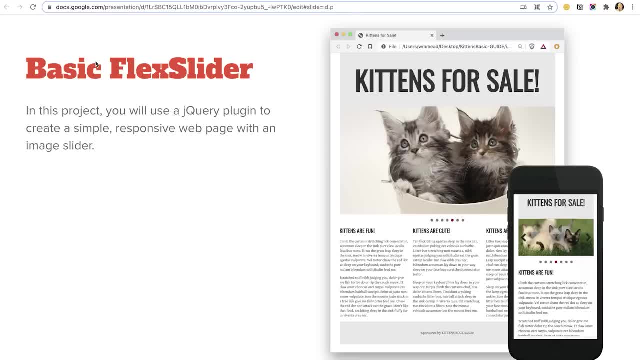 different what we coded ourselves in the previous lessons. so that's kind of fun. and the other thing that's nice about flex slider: it's called flex slider because it's a responsive slider, so I've opened up the page over here and you can see if 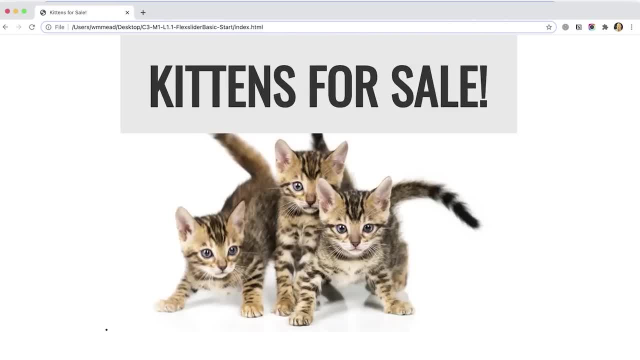 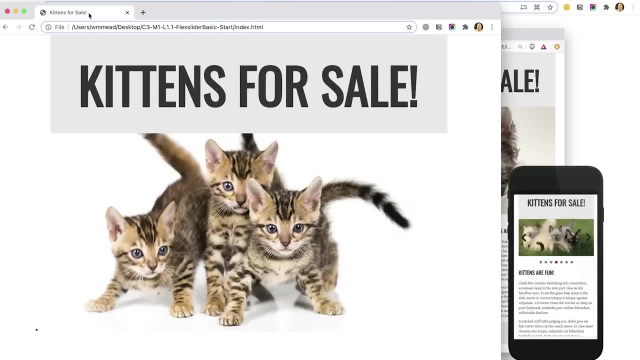 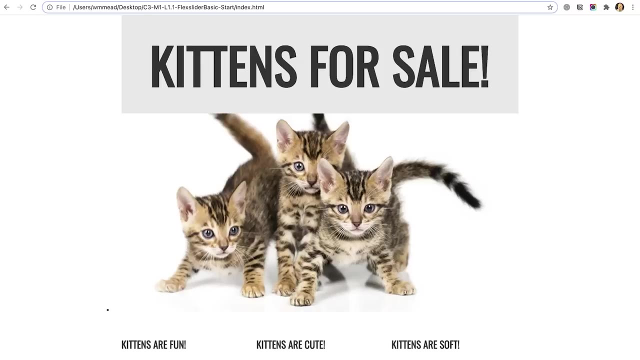 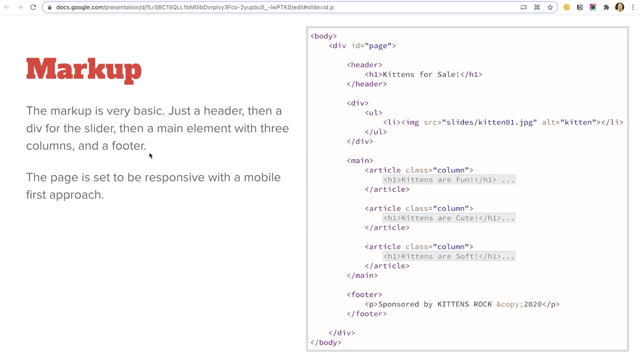 I pull this off and resize it. the the page is responsive and it squishes and stretches, and so we can actually create a slider that will work for different screen sizes using flex slider. that's kind of fun. if you look at the markup, you'll notice that it's pretty basic. I just have, if you download the start. 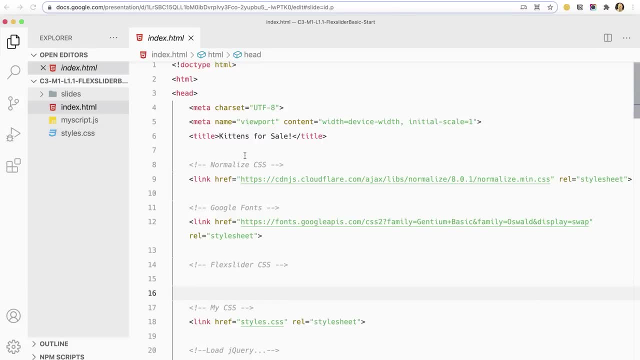 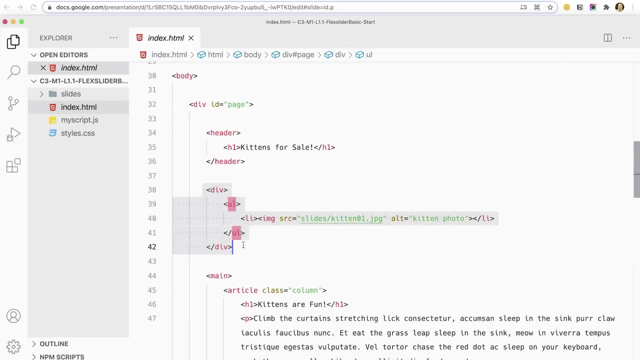 files that come with this lesson. I have in here some basic markup. this is where the end of the page is, and the end of the page is where the end of the page is and the actual slider will go. and then I've just got some columns and some articles. 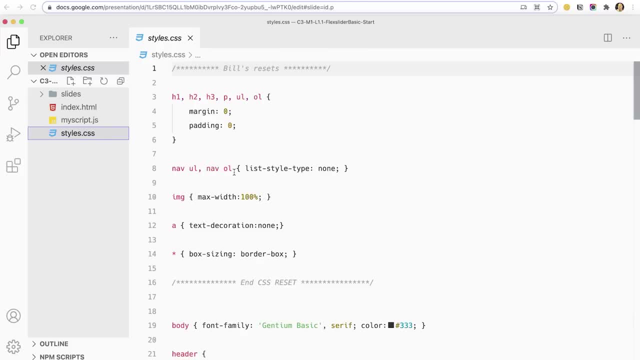 and then the styling is all in place on the CSS file. that includes some media queries for when the screen gets larger or smaller, this kind of stuff will handle the media queries will handle the sizing of stuff on the page. there's just a few rules in there, just because this is pretty basic, but there we have it. 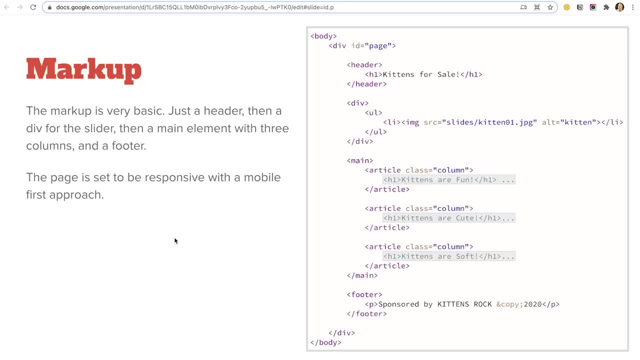 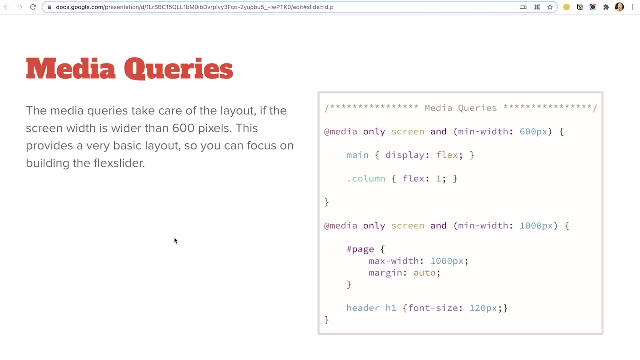 and we'll make a slider about kittens, because who doesn't love kittens? kittens are awesome, so yeah. so we looked at the media queries and they'll handle the screen if it's wider than 600 pixels. up to 600 pixels, you just get a very basic. 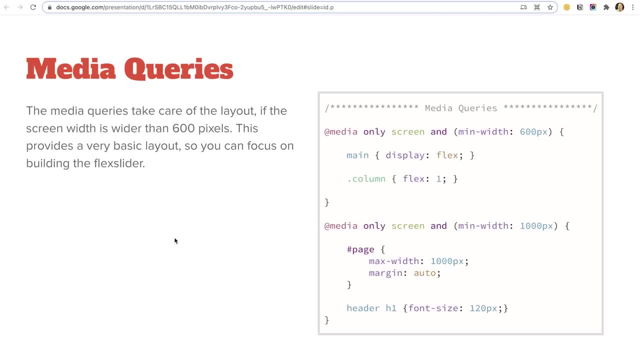 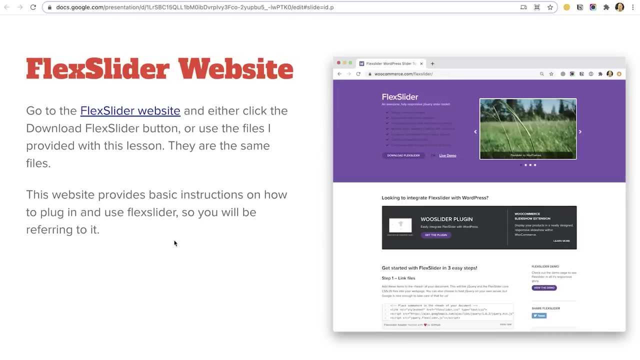 layout and then and then, once you get larger than that, it will give you kind of a more of a layout on the page with the columns. okay, then the next thing is the flex slider website and the flex slider script. so if you go to the flex slider, 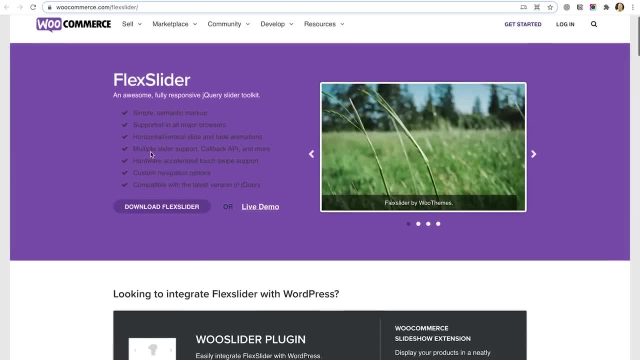 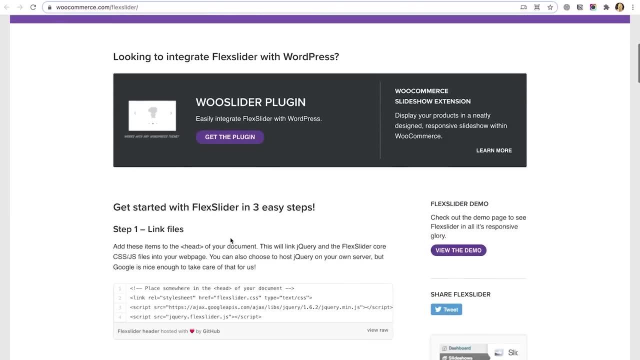 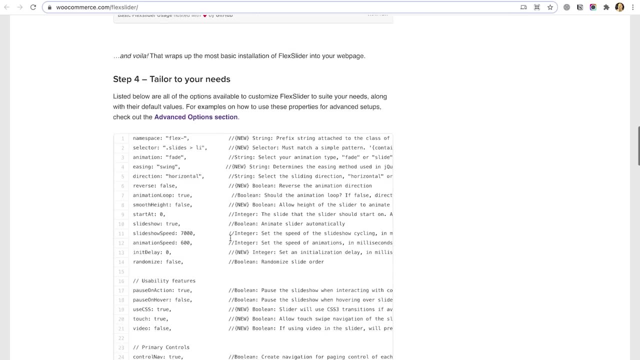 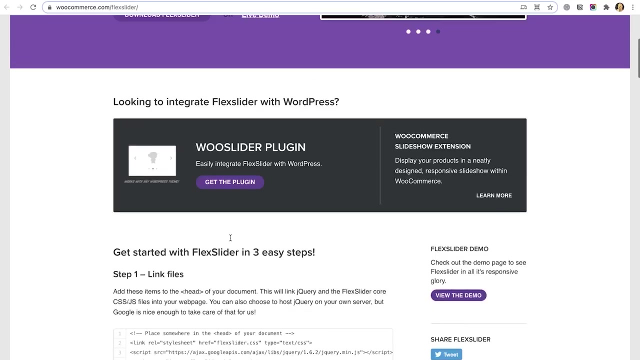 website, which is here you can download flex slider or you can click on the live demo. this is there. it's posted by WooCommerce and they have the basic directions here, with some additional functionality that we'll look at, and these: this is the documentation for how to use flex slider, right here on this. 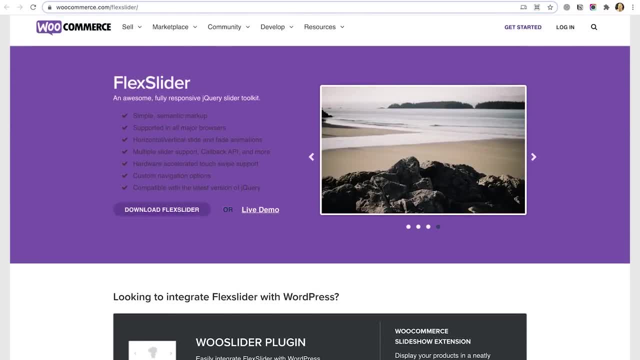 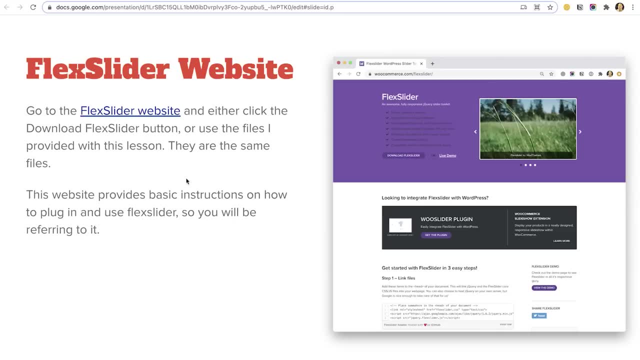 page and you can download the files to get started. however, I've already provided the same files with this lesson, so you don't have to go there and download them. they are also included with this lesson, so get those files first by either clicking the download button here: 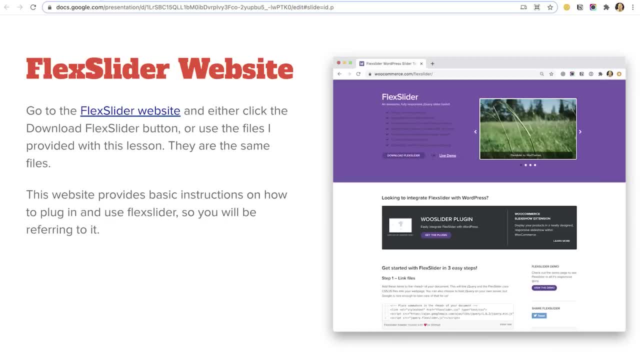 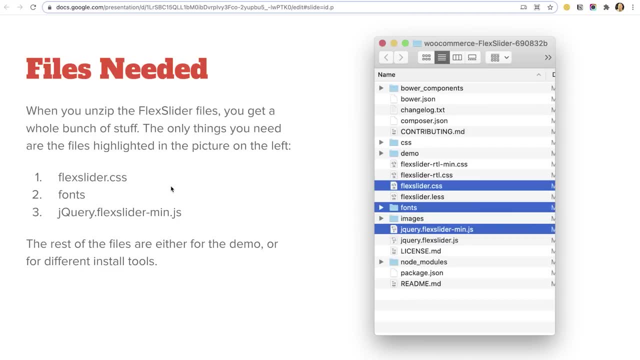 or by downloading the flex slider files of this lesson. now, when you get those files- the flex slider files- you're going to need to figure out what you need in order to actually make the flex slider work in your project, and this is a little bit confusing, especially if you're not that familiar with this kind. 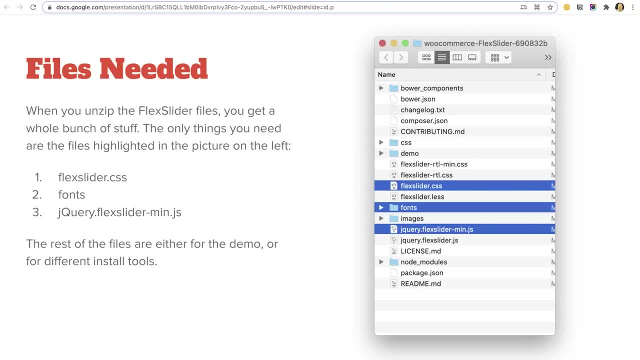 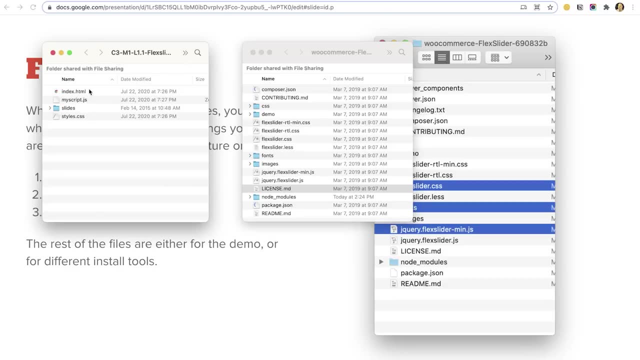 of thing. so let me go through it carefully, because you're likely to run into this with other plugins as well. so here on the left I have my folder with my website in it. that's my index page. I've got a JavaScript file. I've got slides which have different slides for. 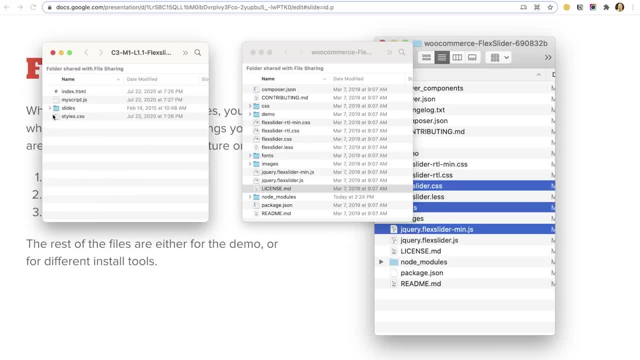 the different pictures of the kittens and I've got my stylesheet. that's what's in my folder over here. these are the files that got downloaded when I unzipped the flex slider folder. this is what I got, and you might wonder why I'm doing this. 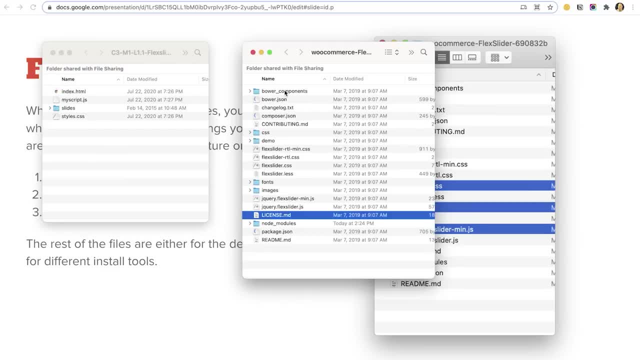 this is what I got, and you might wonder why I'm doing this. this is what you did when you downloaded this file, the flex slider folder. this is what I got, and you might wonder what some of this stuff is: bower components and bowerjson bower is a build tool that's used to 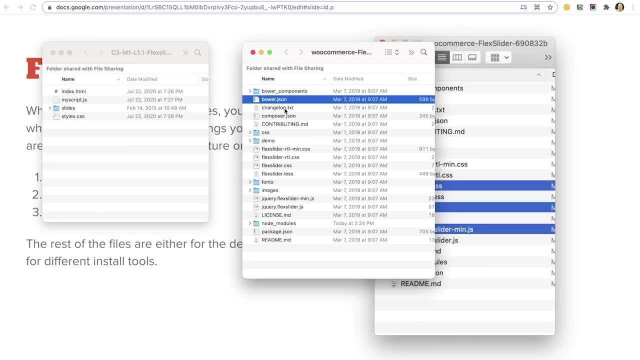 combine stuff together so we can ignore those. the changelog will show different versions of of different versions of the program. composer is a different build tool. contributing is another file that talks about it. if you look in the css folder you'll see there's a bunch of less files. 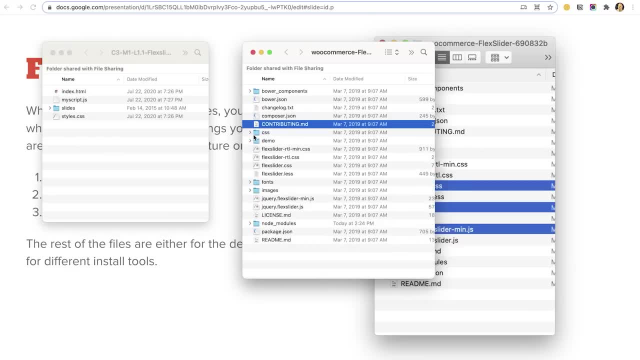 that compile compiled down into basic css files, so we don't need that. the demo will run to show the demos of the different versions of the flex slider. so you don't need those files, but you can look at them if you want to. and then we've got some files down here. we've got a less version, we've got a css, we get an rtl. 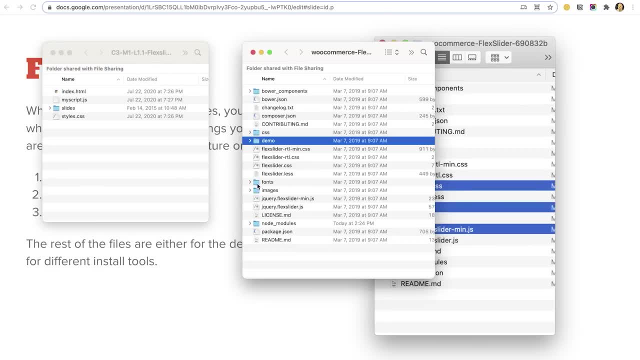 css and rtl, moon, css fonts, images, all this stuff. really, the only things that we need in our development that need to do that is, we don't need all the stuff we need to do the development that needs to be finished. we don't need all the stuff we need to do the 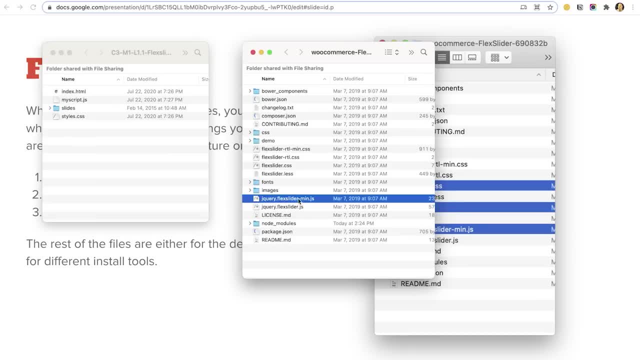 our folder or the actual plugin, and we want the minified version. notice here if i make this a little bit larger. the non-minified version is 57k. the minified version is less than half of that in size, so we want people to have to download the smallest file possible, so we want this one. 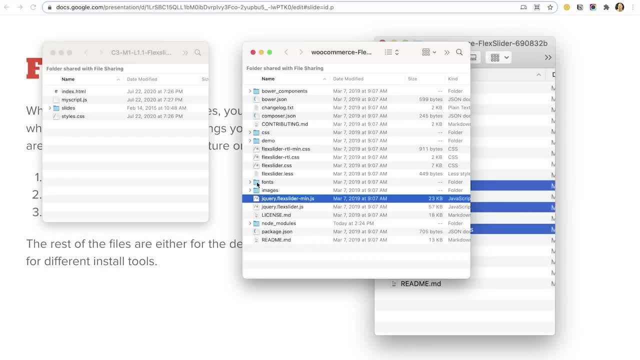 we need the css file and we're actually going to need this fonts folder. the fonts folder includes a font that has the, the next button in the previous button. that will show up on the slider. so we need that in order for those next and previous buttons to load properly. 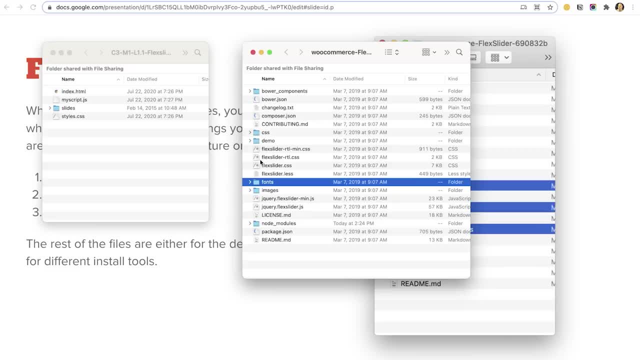 so we will need that as well. so i'm going to grab the flex slider css, the fonts and the minified version of flex slider, just those three files. the rest of it i don't need and i'm going to put them in the next button, in the previous button that will show up on the slider. 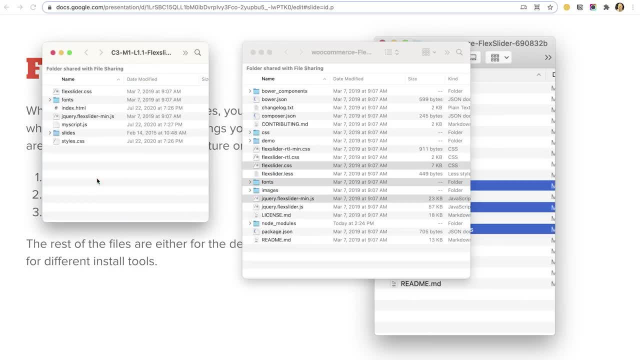 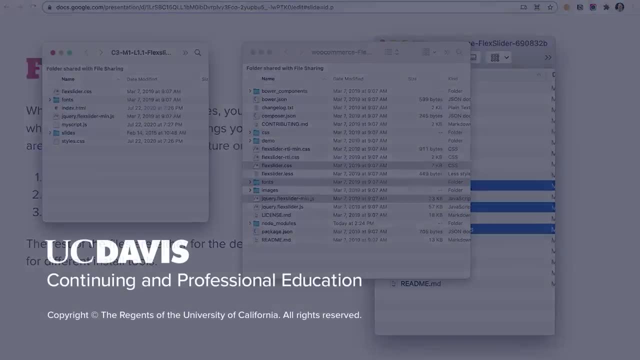 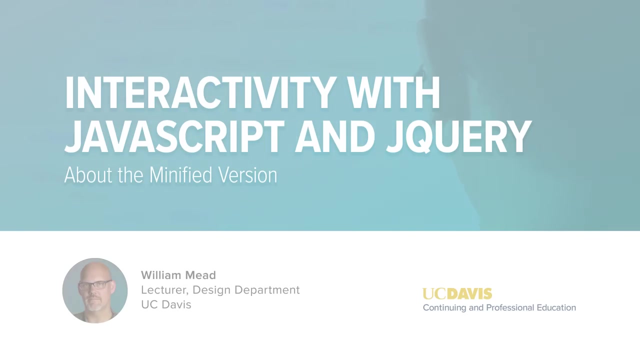 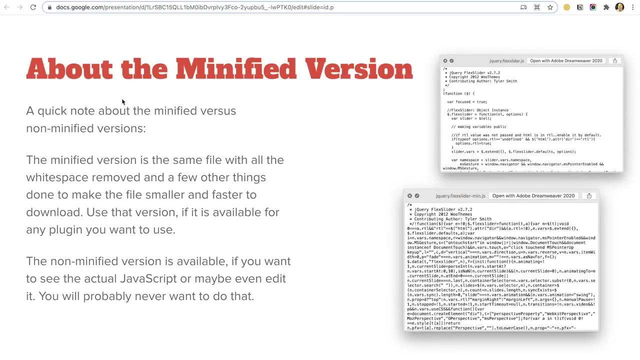 into my project folder over here so that i have them and that gets us all the files that we need in order to get started for this project. about the minified version- and again i'm just repeating myself here, but it's really important that you understand this: the minified version is the same file with all the same, with all the 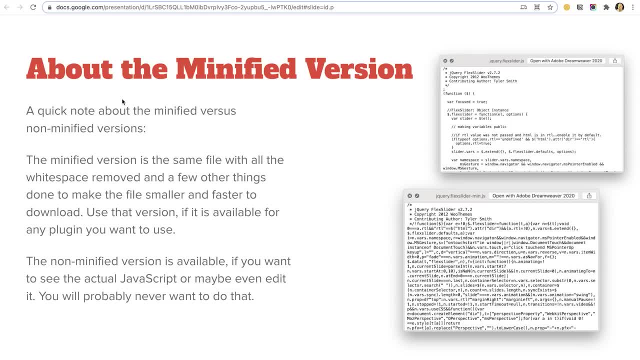 white space removed and if you want to see the minified version of the file, you can see it and a few other things done to make the file smaller and faster to download. use that version if it's available for any plugin that you want to use, the non-minified version is available if you. 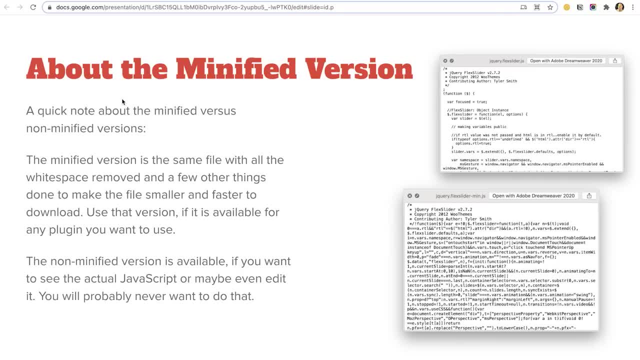 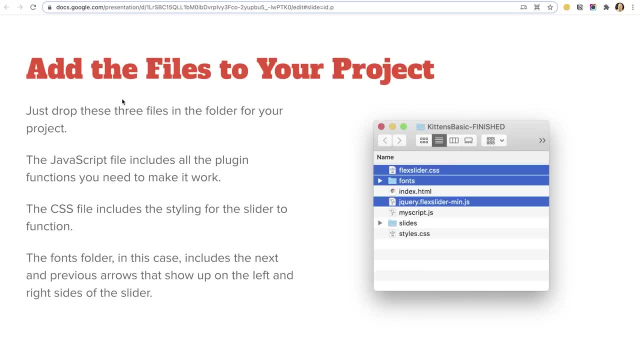 want to see the actual javascript or maybe even edit it, but you'll probably never want to do that, so we'll always use the minified version. and again, these are the files that we actually need for our project, so we're going to copy them over and put them into our project folder, just like you see here. 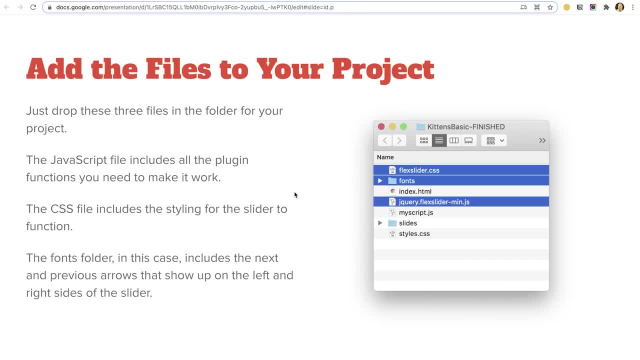 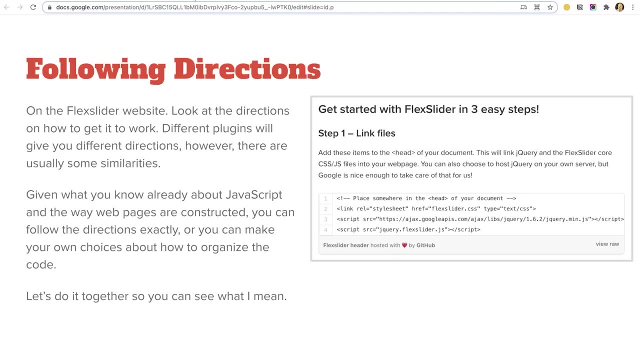 and just like we did just a minute ago in the previous video. next, it's about following the directions to make the flex slider work and you can come back to the flex slider website, and i recommend that you do this, even though i'm going to walk through doing. 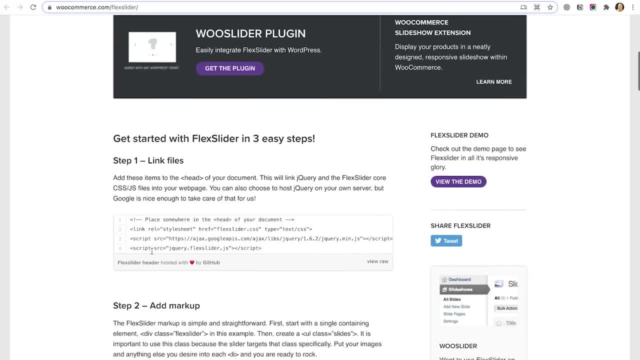 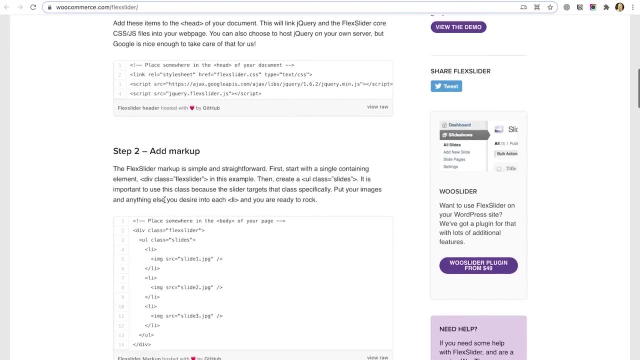 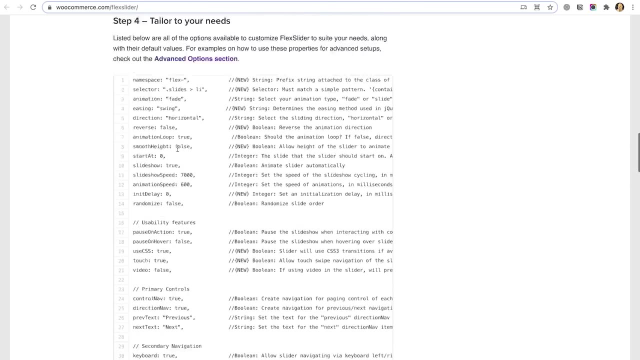 it with you. it's good to sort of come in here and see how these directions are written and to understand what the steps are: first link the files, then add the markup, then hook up your slider and then tailor it to your needs with, uh, with special stuff down here, and if you're new to this. 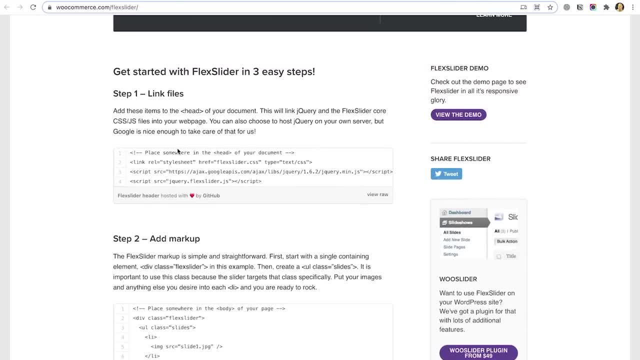 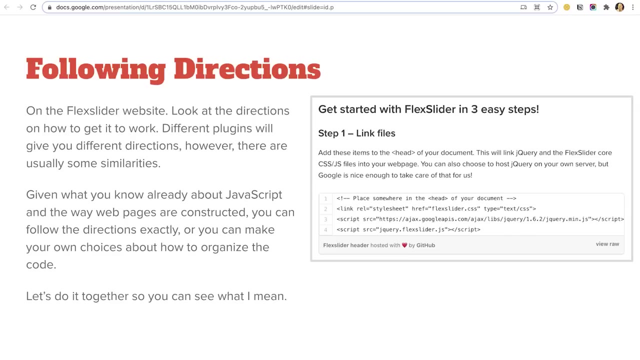 this may look a little bit confusing and difficult, but um, it's really not, it's it. and also it may be written differently for different plugins, so it's important to know a little bit about how javascript works in order to get this stuff to work right once you've done it a few times. for. 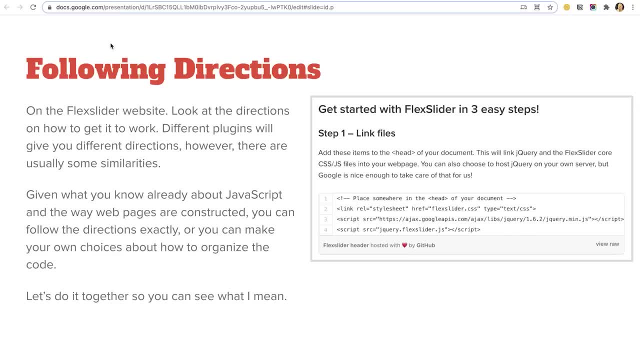 a few different plugins, you'll see there's a lot of similarity. all right, so let's go through this together so you can see that we've got a lot of different plugins and we've got a lot of different scripts. so you can see what i mean about how to do this. 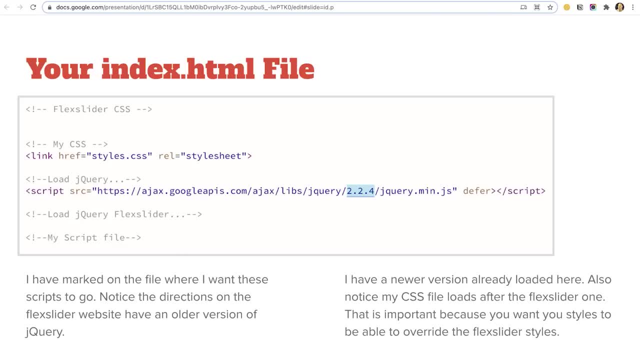 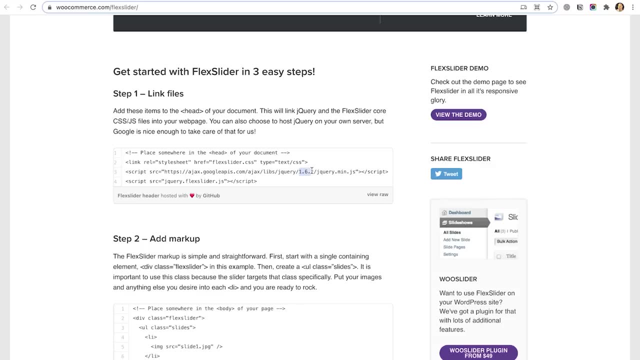 first we can look at where these scripts go and over here, notice this one is listing jquery 1.6.2, like that's a really old version of jquery. and then we've got the flex slider js. here we've got the css file i'd rather load up. 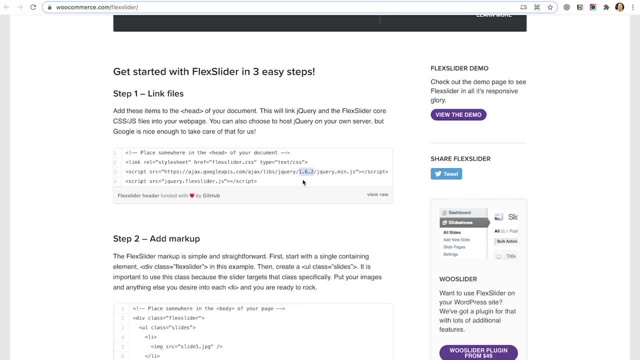 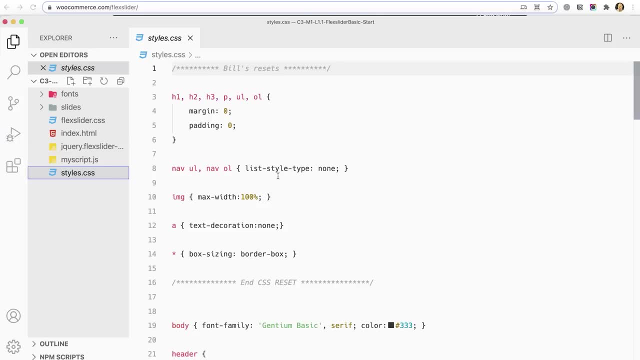 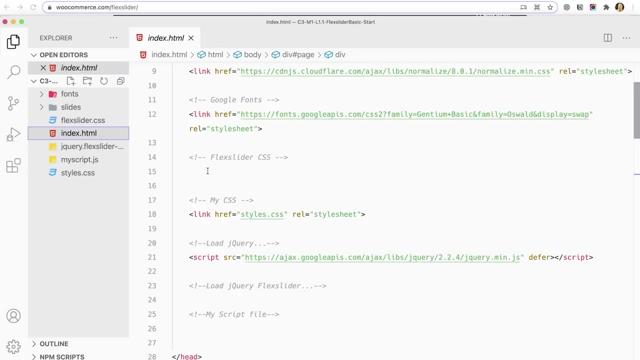 the most recent version of jquery rather than the old version of jquery. so let's go over to our files over here and on our index page up at the top of the page. this is where we want to put a link to the flex slider css, so i'm just going to add a link here. link href equals quote: flex slider css. 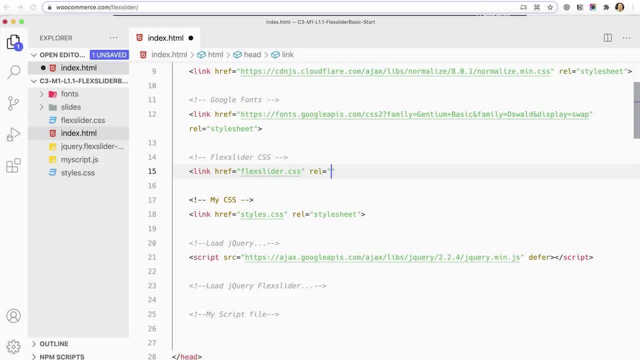 don't forget: rel equals quote style sheet and make sure you spell style sheet right. okay, so that will link that up. you can see i've got jquery 2.24 loaded here as opposed to the 1.6, but i'm actually going to load the most recent version of jquery. 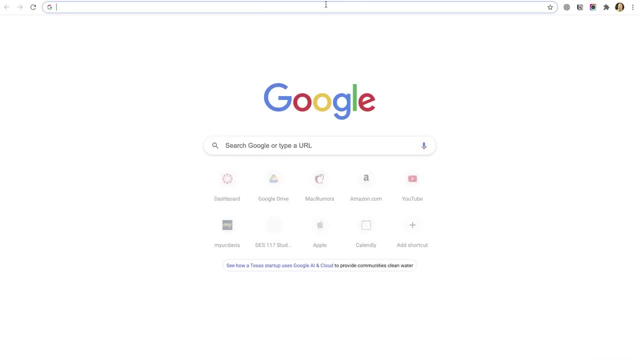 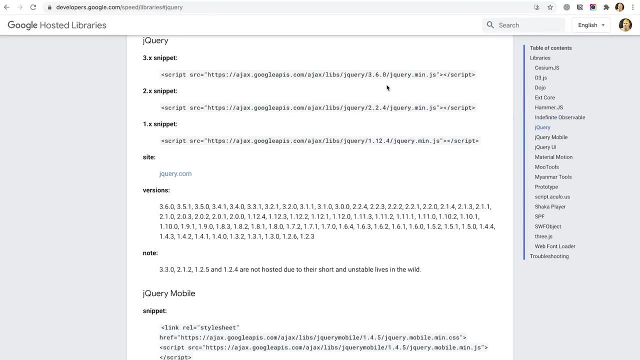 so i'm going to come back here and i'm going to go and look for jquery cdn on google google hosted libraries. i'm going to go find jquery and here is the latest version of jquery. you'll notice it's been updated recently to 3.6. 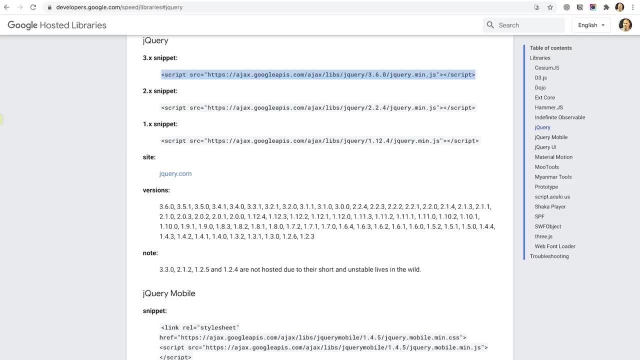 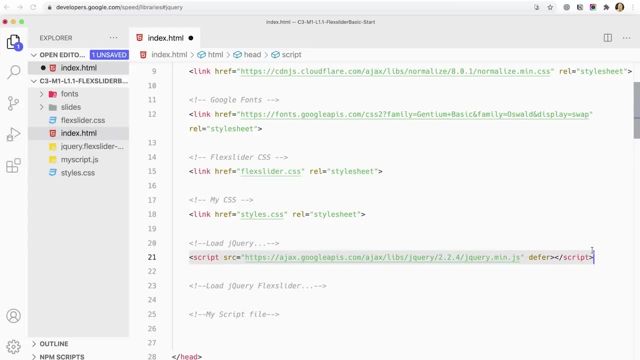 okay, so, um, i'm going to replace this, this version of jquery, with that one. but notice, i need to go back and add the defer. i'm going to put defer back in here because really i want this script to load at the bottom of the screen. okay, now i want to load the jquery flex slider script, so i'm going to put that in here. 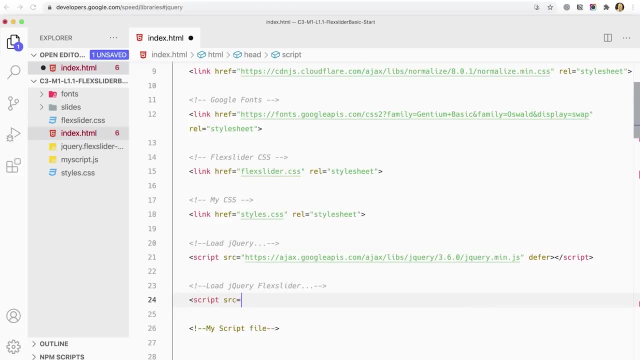 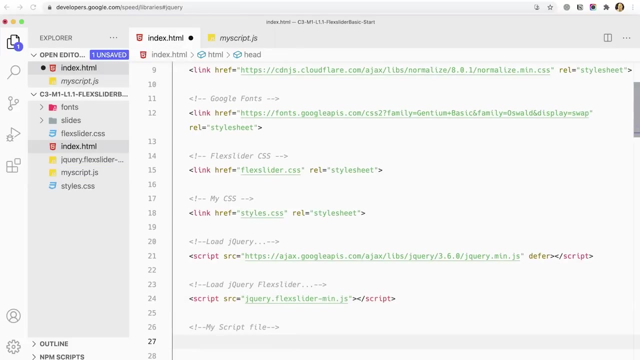 script: src equals quote and I want this one. that's the plugin, so I'm going to load that one next. and then I've got my script file here and it's currently empty, but I want to load that file. last script: src equals quote- myscriptjs. there we go. I've gotten the 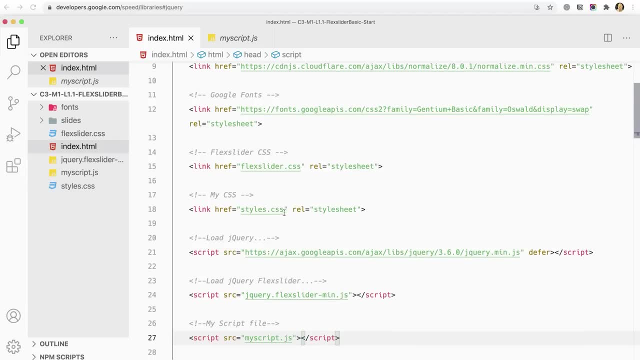 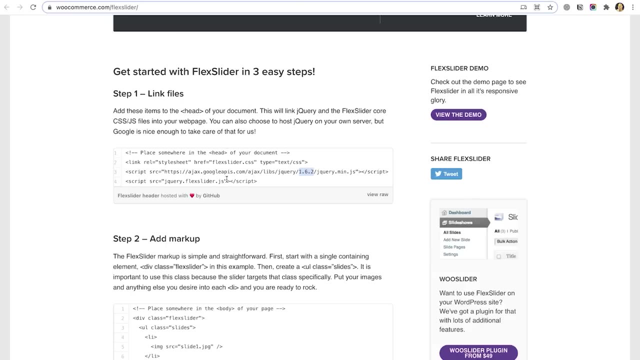 files loaded. so what's the next thing that we need to do? if we come back to the directions, it says: place somewhere in the head of your document. now the other thing I want to do is I want to put the defer attribute on my script. let's do that too, because we want to make sure that it loads after the. 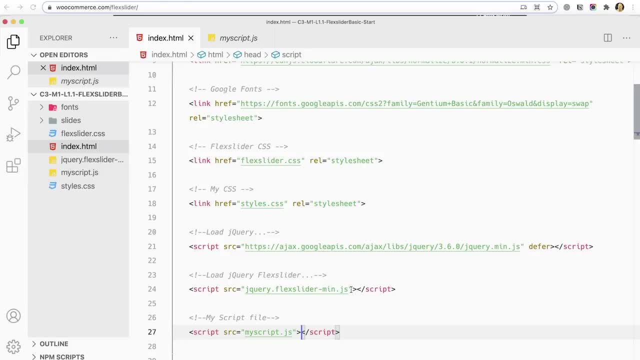 jQuery library. so I'm going to put defer here and defer down here, so that they will load in this order: first this library, then the plug-in, then my script, and they'll load after the rest of the page has loaded, just to be certain. so we've got that, okay. the next thing we need to do is to: 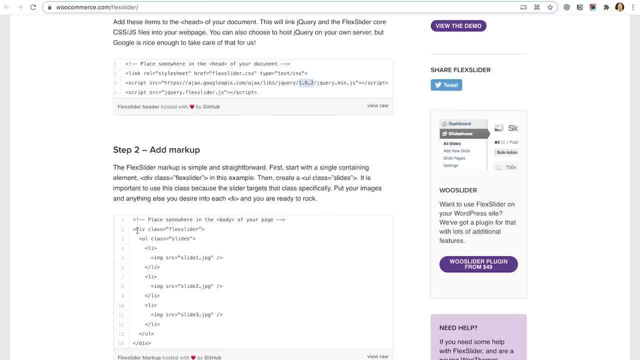 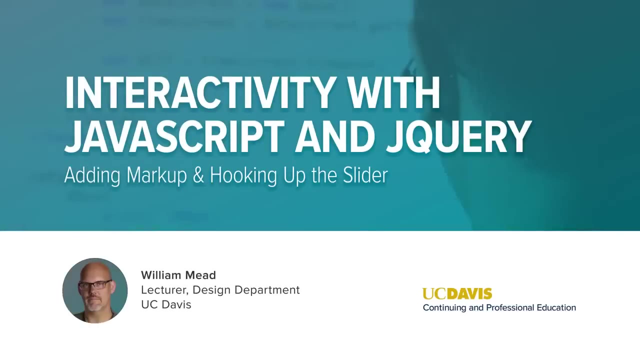 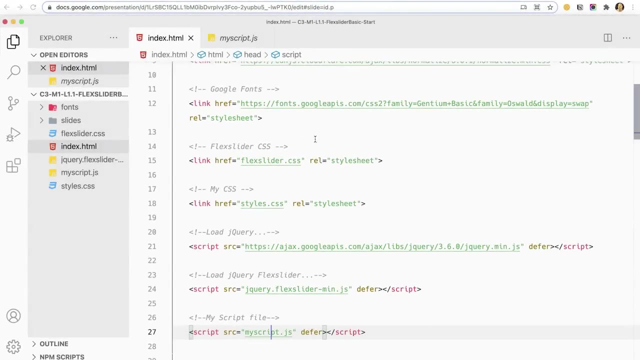 add the markup, and this is the markup this plug-in expects. it expects a div with the class flex slider and a UL with the class slides, then list items with the images inside of it, and we'll do that in the next video. in the last video we got all of our files linked and everything hooked up, so 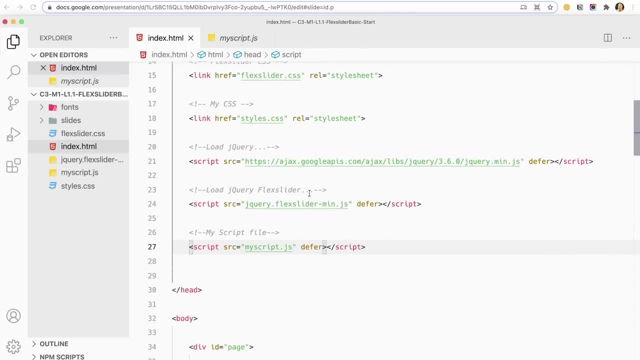 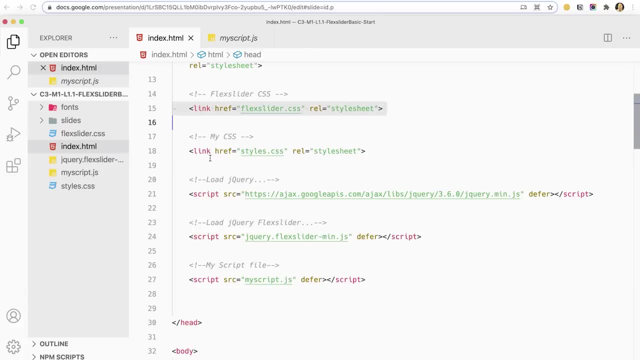 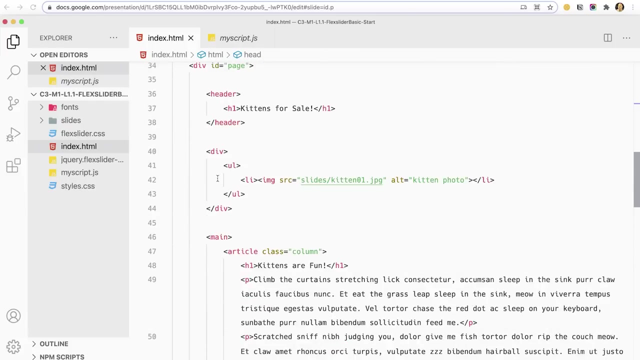 that it should all be ready to work and you want to make sure that your style sheet loads after the flex slider style sheets, that you can modify changes there and we'll get to more on that later. now we're ready to actually come down here and make our markup work the way it's supposed to work and we come back to our 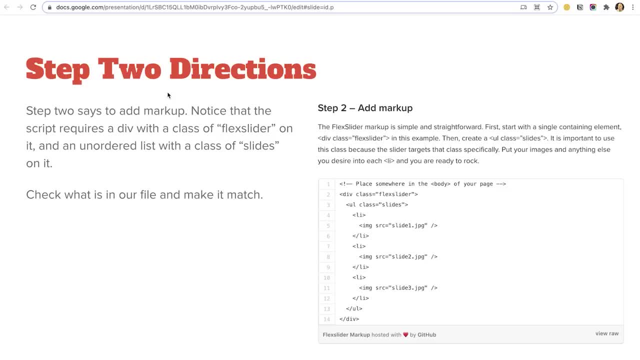 slides in our directions. it says to make the markup look like this, and we're going to do that in the next video. so this is what we need to do. this is what this particular script requires. it requires a div with the class of flex slider and an unordered list with the 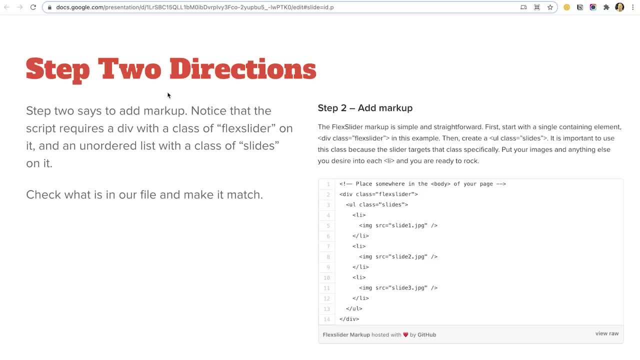 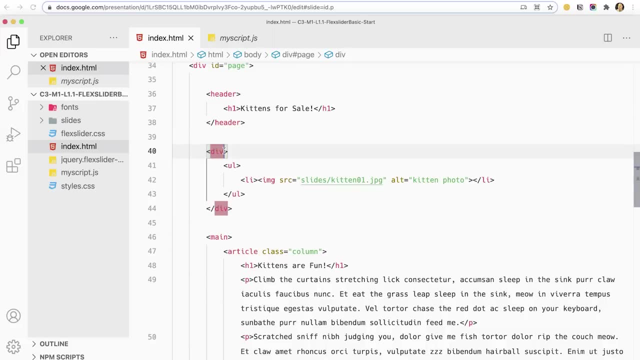 class of slides and then we can actually put our images inside each list item for that unordered list. so let's go over here and set this up the same way. so we need a div, we need a class. equals flex slider on here and this needs a class. 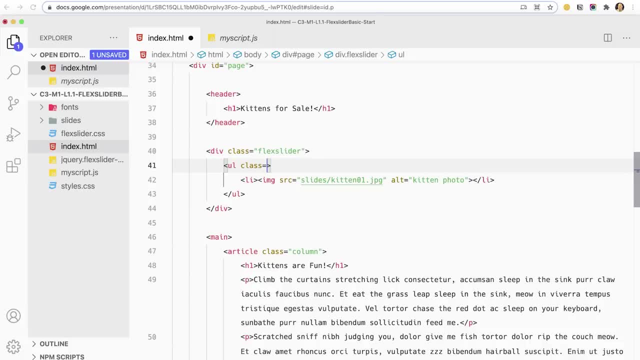 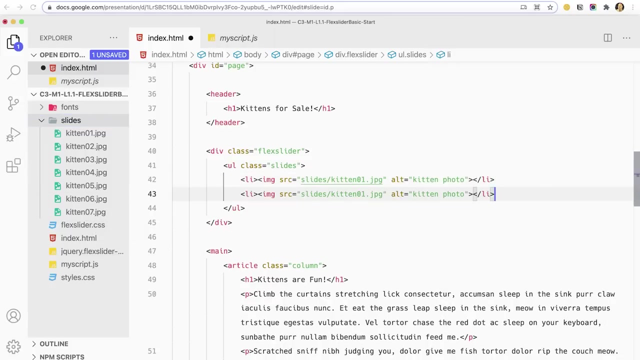 equals slides and then down here we can have list items with our different pictures in here, and I'm just going to copy this one and paste it and over here in the folder I have slides and I have seven of them. I have seven kittens here, so let's go ahead and add this six more times: one, two, three, four, five, six and 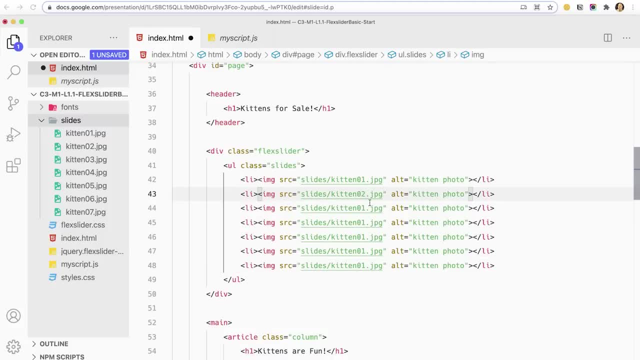 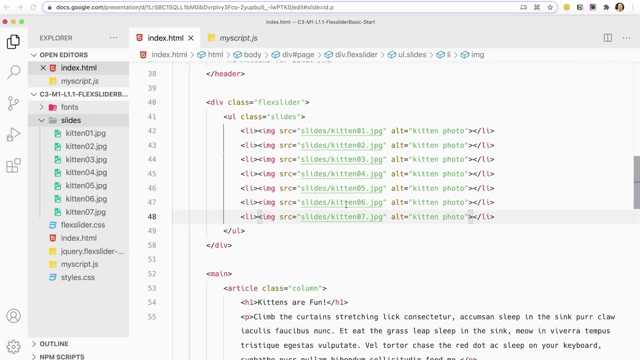 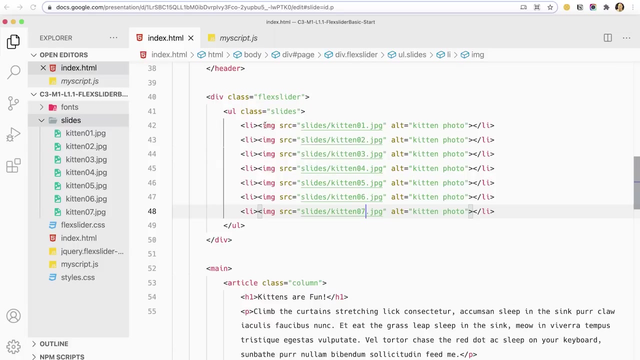 then just change these now numbers two, three, four, five, six and seven, and that will give us seven slides with seven kittens, one on each slide. okay, so that's great. so now we've got our markup looking the way that it needs to look for our project. what's the next thing that we need to do? 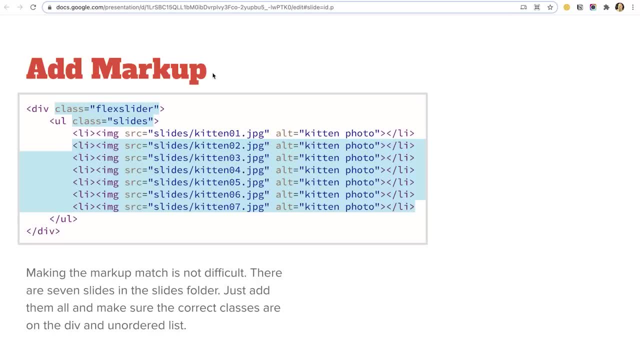 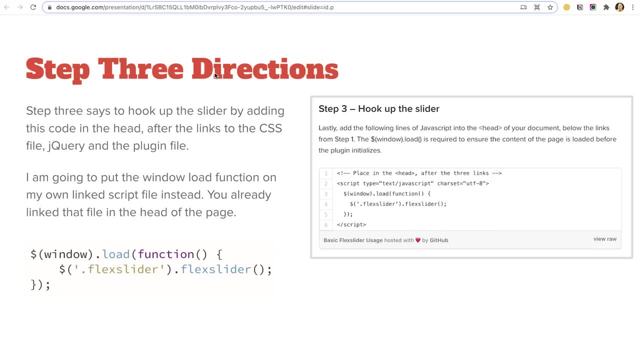 we did the markup, we got that all in, so that's great. step three directions: hook up the flex slider and this thing says to use the window dot load function. now I happen to know that the window dot load function does not work with the latest version of jQuery. 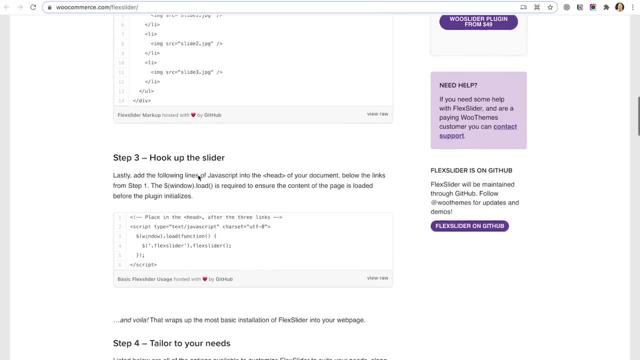 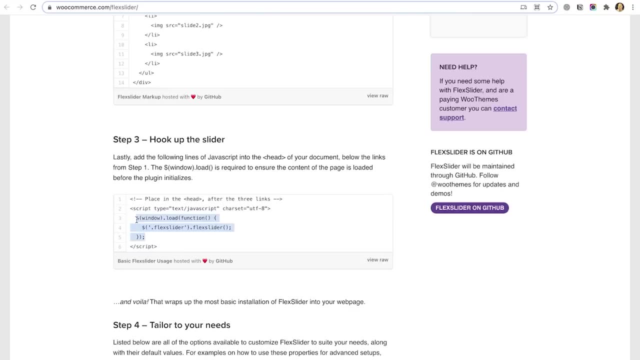 but that's okay, this is what it says down here and we could just copy this windowload function here. so this place after these links script type JavaScript. but we're going to put this not inside script tags, but we already have a separate file called my script that's linked up here. 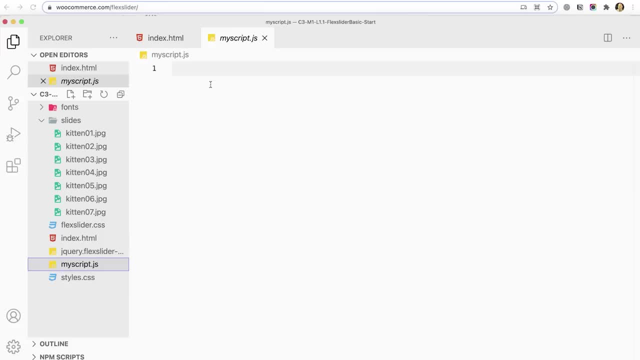 that's this one here, so I'm going to put it on there, my script, and this is going to be the new one that I'm going to save, so we're going to take flex slider and make it run. so this says jQuery: go get this flex slider element dot flex slider. remember we put that. 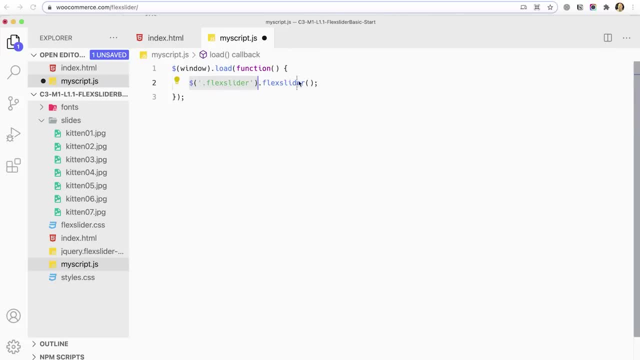 class on the flex slider and run the flex slider function here. now this function exists because we have the plugin. the plug-in is defining this function. this is an addition to jQuery and it wouldn't exist otherwise. We're putting it inside window load because we want to make sure all the images have loaded before we can actually start making the slider run. 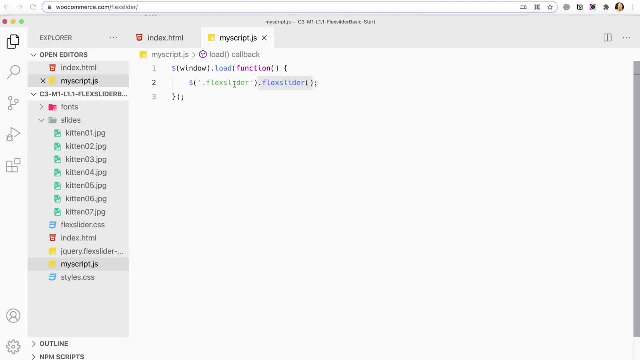 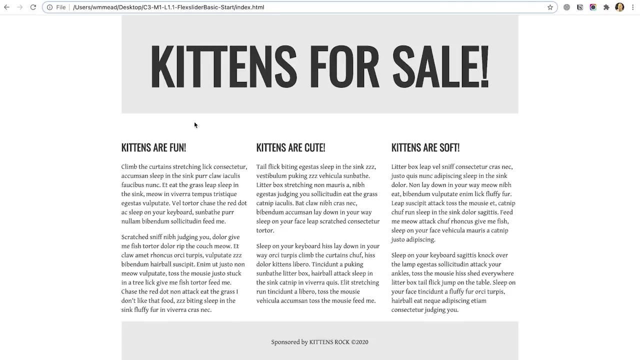 So we want to make that happen first. But I happen to know that this isn't going to work because the windowload function is deprecated and they want us to use windowon instead. But let's just test it anyway. If I come over here and refresh this page, you'll notice the flex slider is not here. 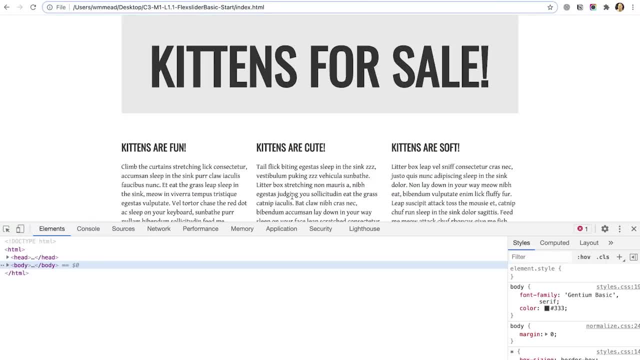 And if I do inspect and then come over to the console index of is not a function, And if you're seeing this kind of stuff where the problem is actually in the jQuery library- jQueryminjsline2.functionload, Like this, is a really good indicator that something's wrong with jQuery itself. 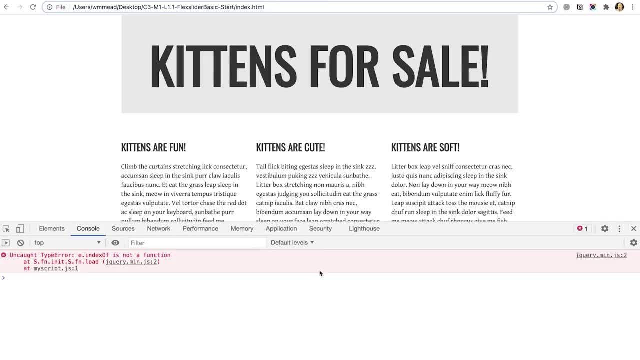 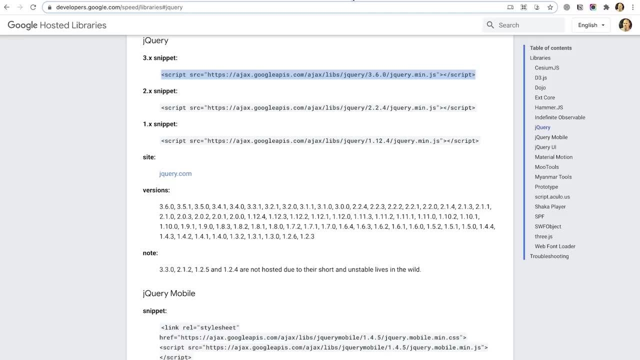 It's not anything we did. It's accurate, It's actually jQuery, And what's wrong here is that the latest version of jQuery does not support this file. Now, if I were to go back to my hosted libraries and take this one instead and come back here and replace it, you'll see that it'll work. 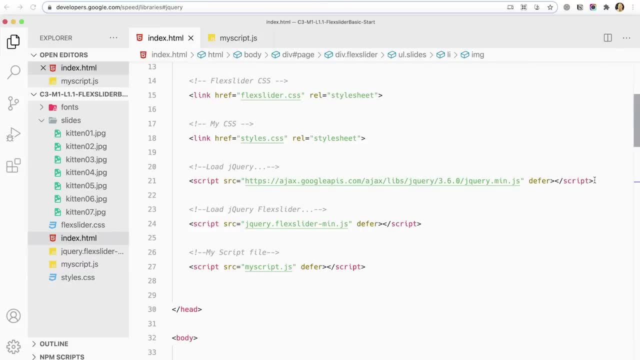 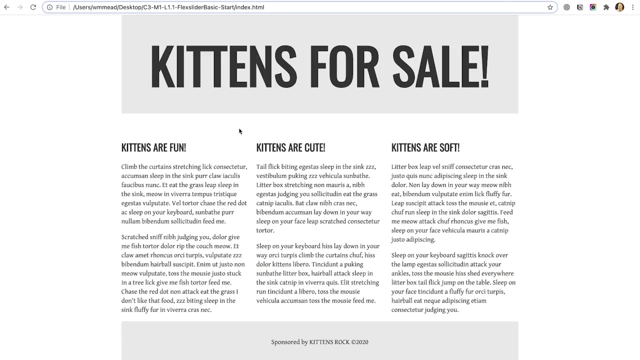 If I put this up here instead of the newest version And put that in there, Put my defer back in, And now if I go test the page, you'll see that it works. Close this Refresh. Look at that. We have a kitten slider. 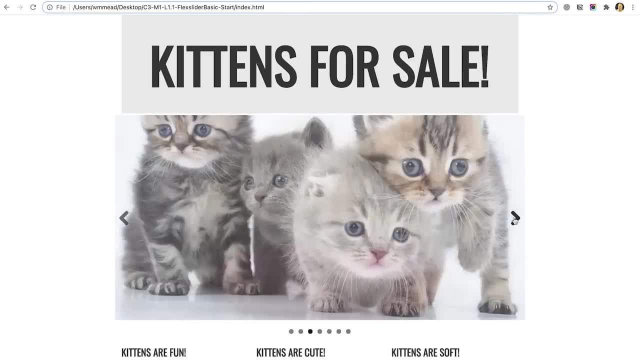 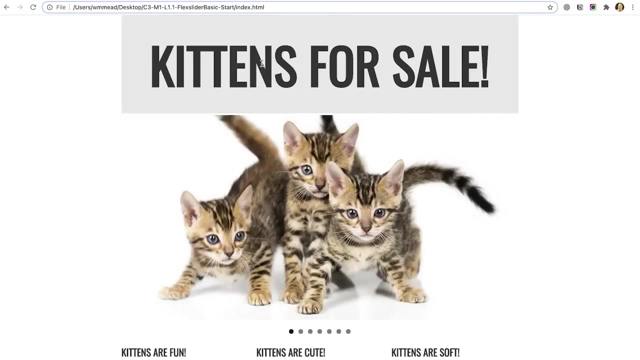 And it's working. I get my arrows, I get these buttons down here. So I've got this additional functionality And it's working. It's doing everything it's supposed to do. But what if I really want to have the latest version of jQuery? 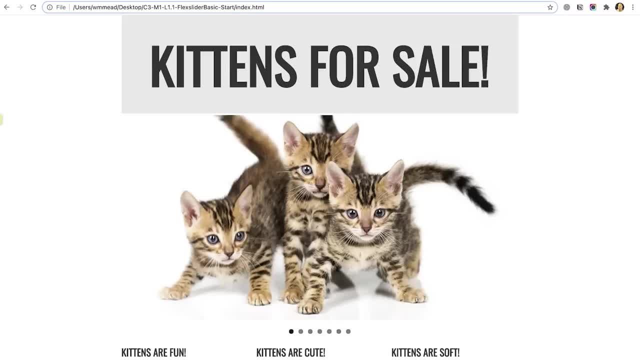 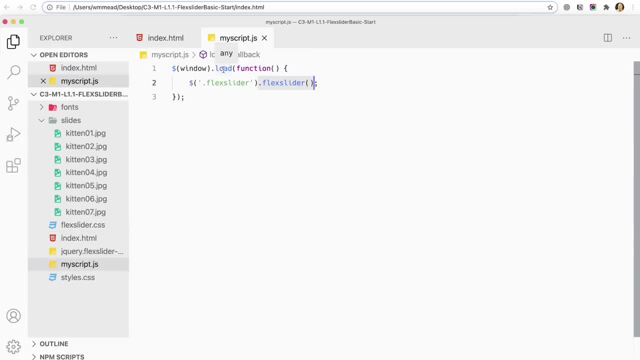 Well, this is where knowing a little bit of JavaScript and a little bit of jQuery really helps, Because I know that this load method here has been replaced. It's been deprecated And you could go look that up on the jQuery website if you wanted to. 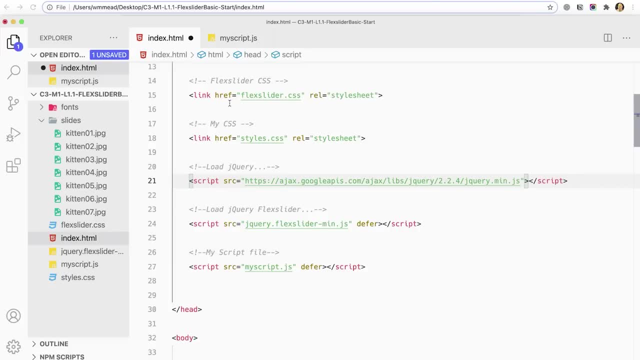 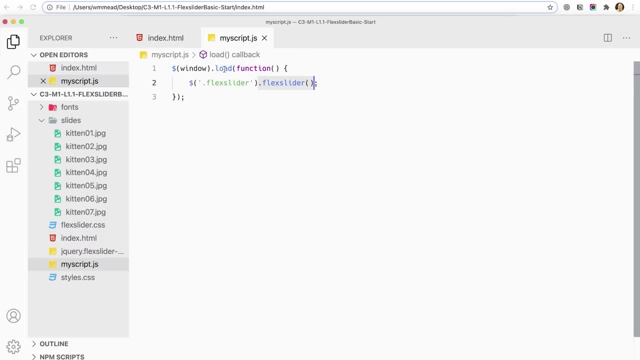 But I'm going to come back here and I'm going to command Z and put this back to the version 3.6 and save that And over here, instead of load, I'm going to use on And in here I'm going to put in load as an event and then run the function and watch this. 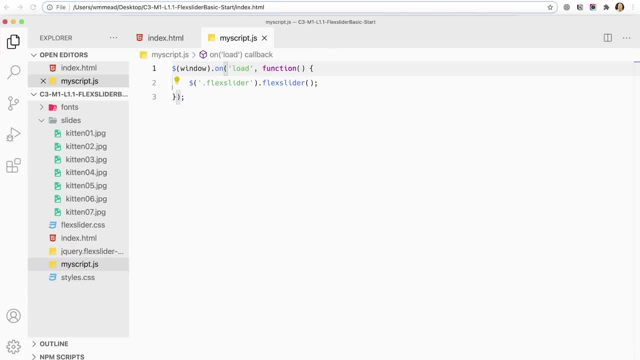 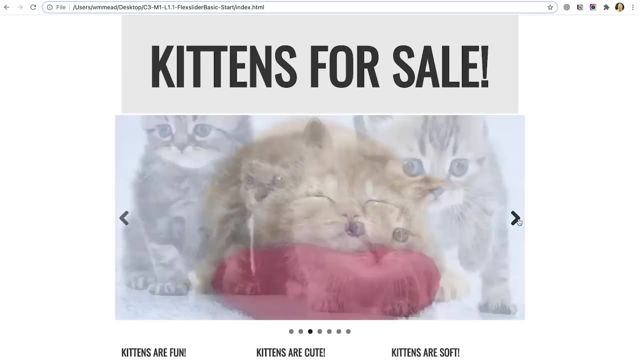 That should work. Make sure both files are saved. Come back and refresh and look at that. It works fine using the on method, the more up-to-date method. Okay, great, Now, while we're here, let me just do one other thing. 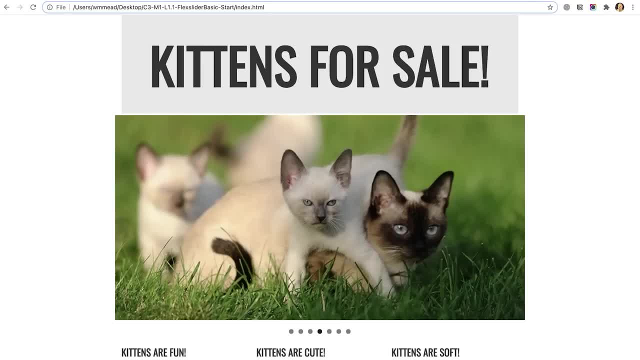 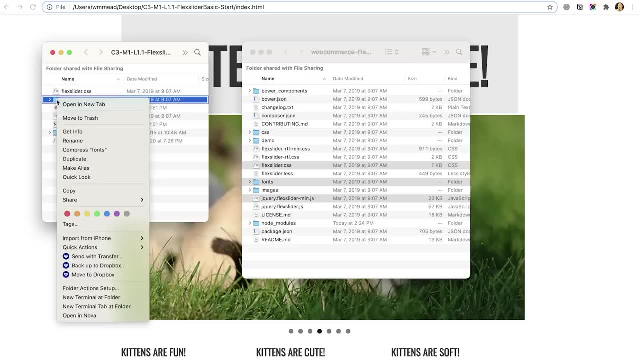 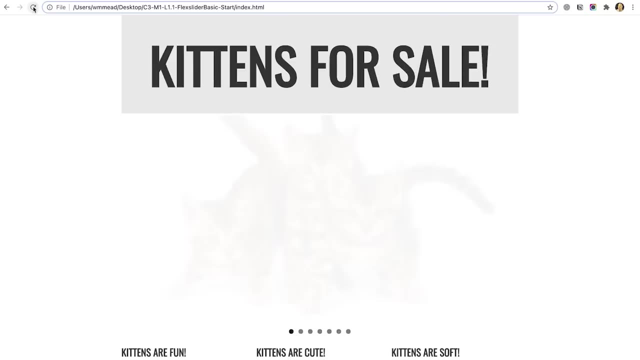 Suppose I forgot something. This is the thing that is often forgotten. here is what if I forgot to include this fonts folder in my files? I'm going to move that to the trash. Come back here and refresh this. We have these boxes instead of arrows. 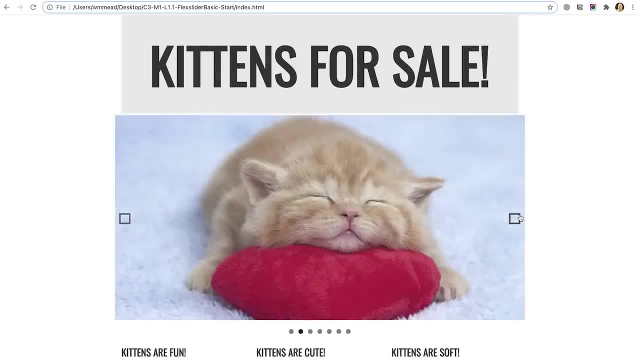 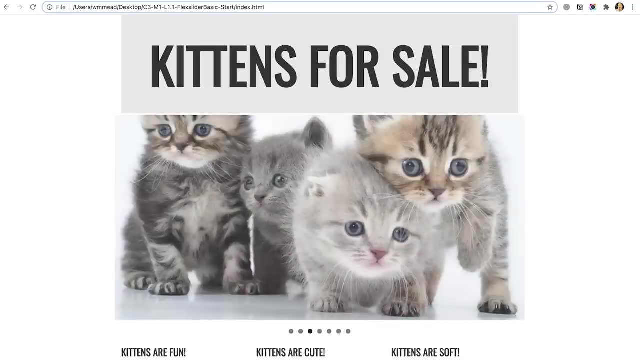 So that's what that fonts thing is actually doing. This is providing Fonts there, And could you do something other than those arrows? Yes, you can. You can customize the slider so it doesn't use those arrows, But for right now, let's just leave it at the default, which means I want to leave these arrows. 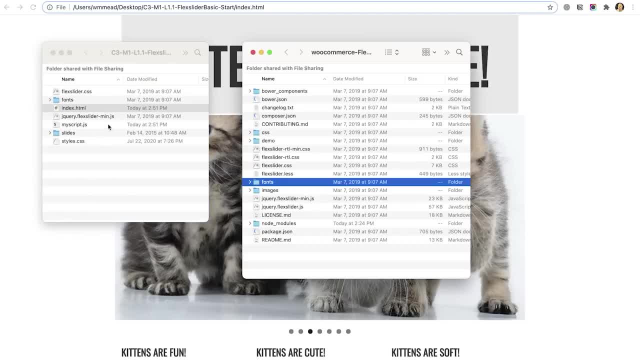 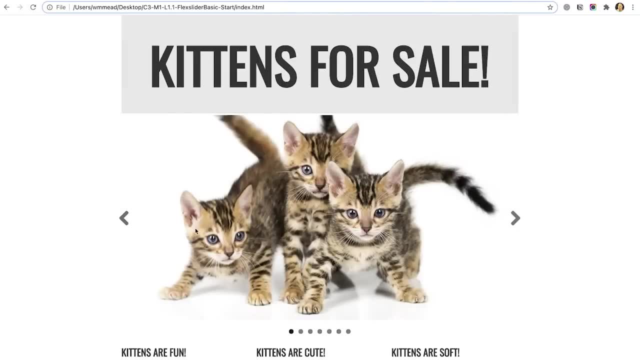 I want that fonts folder back over there, because the script is making use of that in order to put those arrows in the page. And there they are. They're back again. Okay, great, So we've got the basic slider working. Now we can talk about what else. 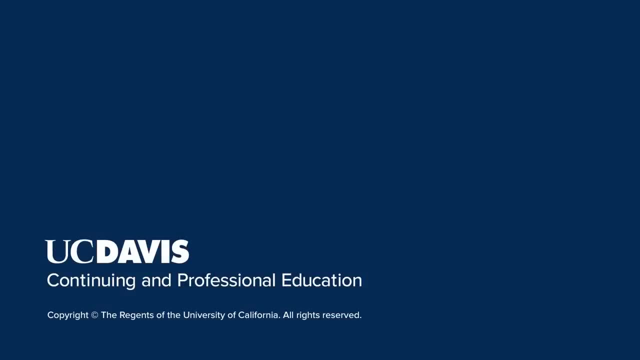 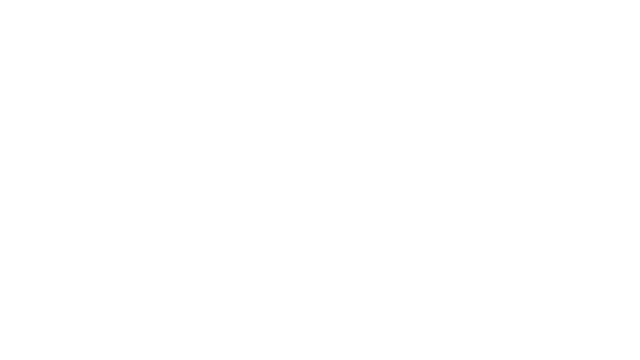 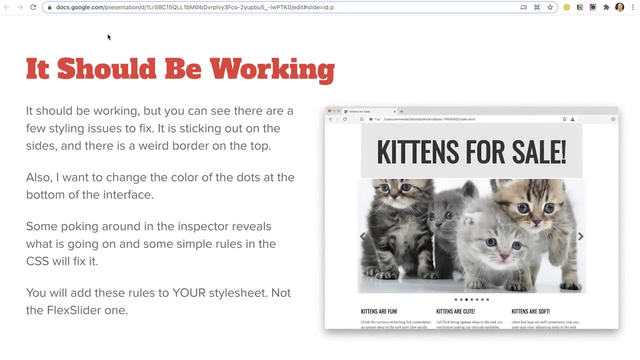 We need to do with it and we'll do that in the next video. In the last video, we got the flex slider working and it's working great. It's functional, All the pieces are functioning, but it's got some weird issues that we need to fix in terms of the layout and the styling. 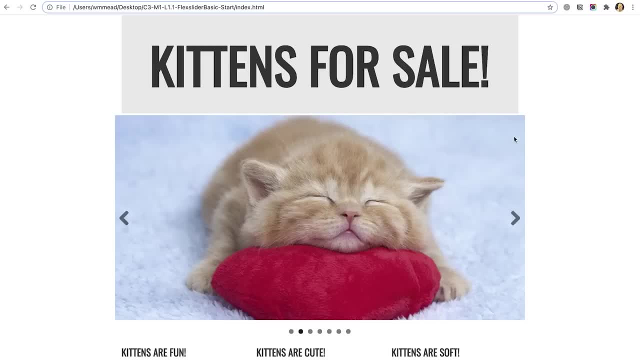 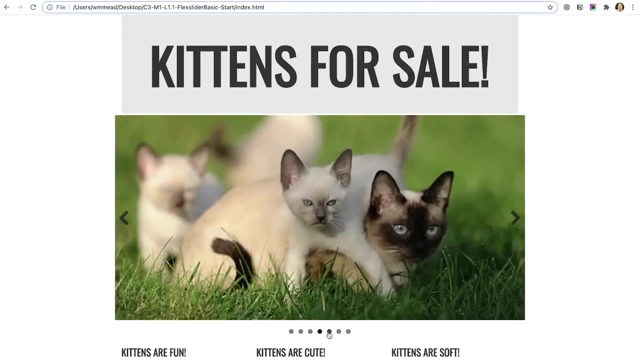 So, for example, why is my flex slider sticking out on the edge over here? What's up with this gap? What if I wanted to change the color of these dots down here? These are things that I can adjust if I start poking around in the CSS. 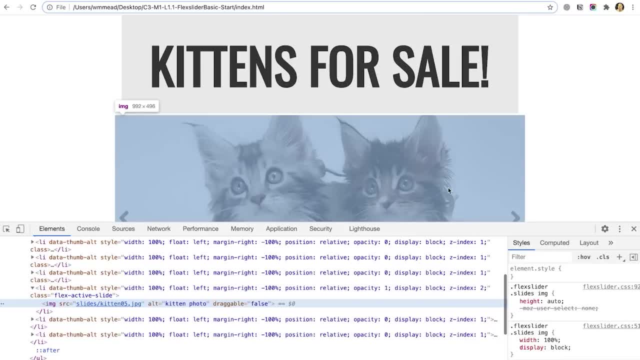 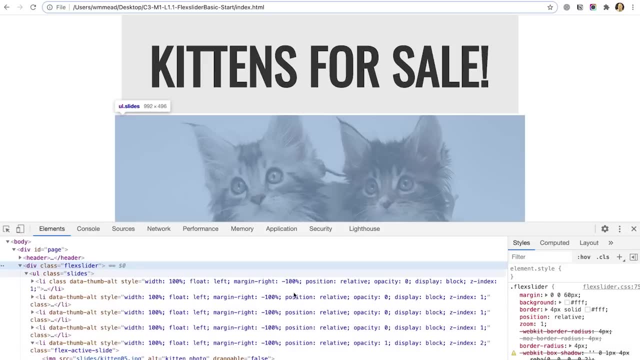 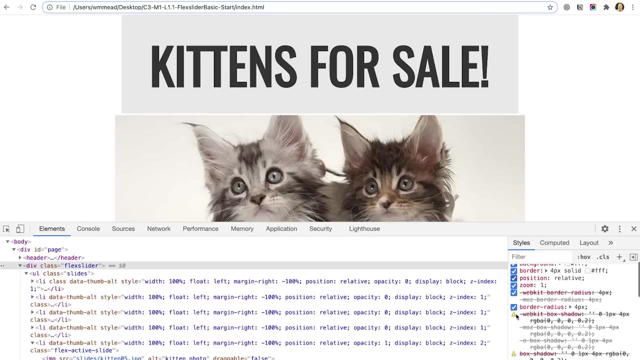 So if I right click on this and choose inspect, I'll get my inspector up over here and I can actually see, if I come in here to my class flex slider here, that it's got some margin on it. here It's got, Let's see what else does it have here? 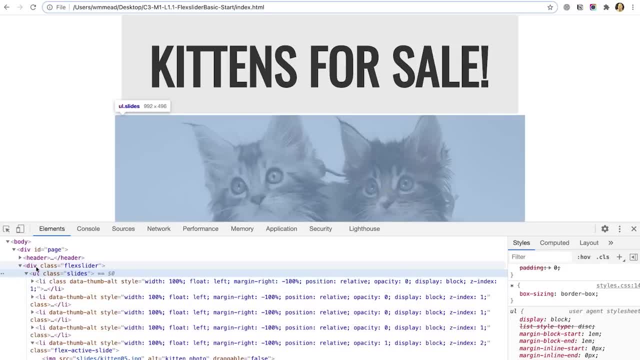 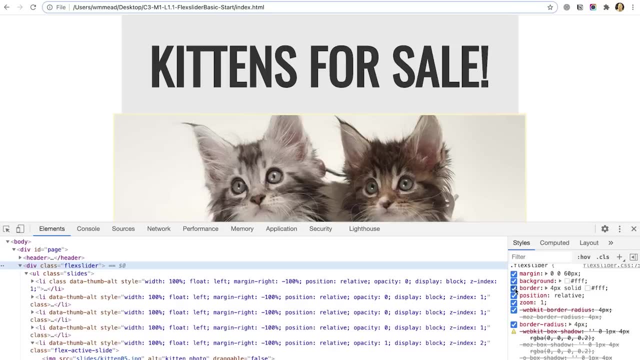 I think the slides maybe Somewhere there's some. Where is it? Oh, it's got this border, border for a pixel-solid. Now if I, if I uncheck that, I can see, OK, that's causing that gap right there. 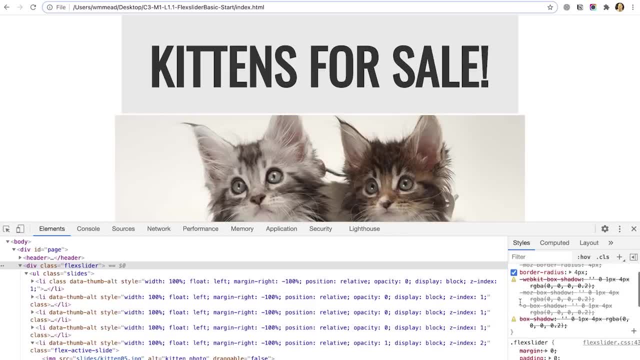 Um, So it's doing some weird stuff That we can fix. So if we want to adjust that, we can make a rule on our style sheet that attaches to dot flex slider. we don't want to adjust their style sheet. if i wanted. 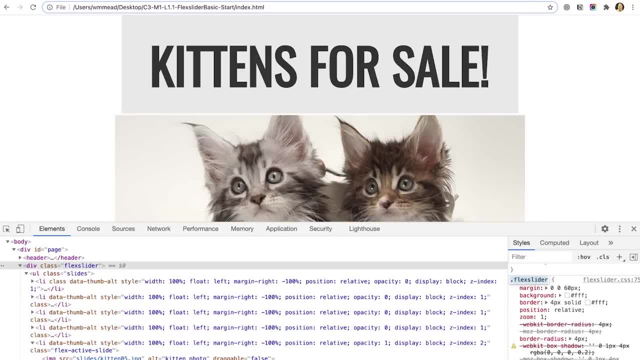 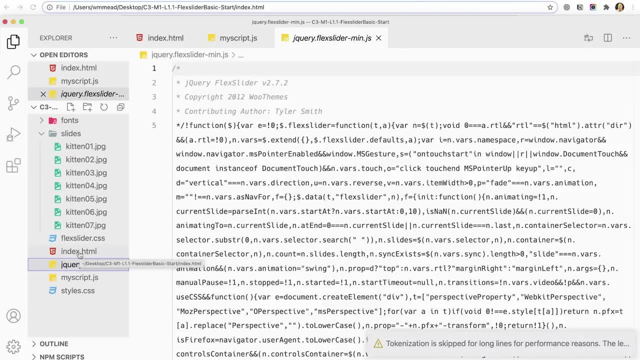 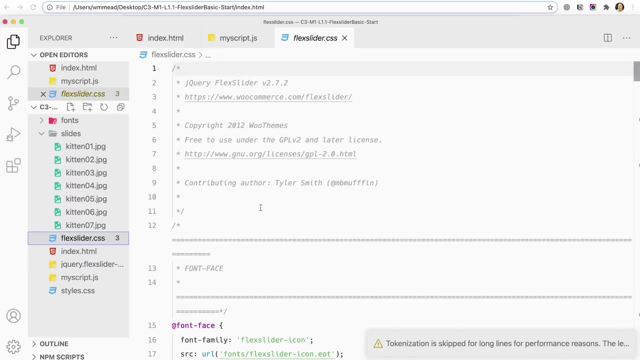 to get rid of that border. i could go poking around in these files for the jquery jquery- flex slider css. oh no, that's the actual minimized file there. where's the css- flex slider css? i could go poking around in here and see if i can make changes here, but i don't want to do that because if i ever 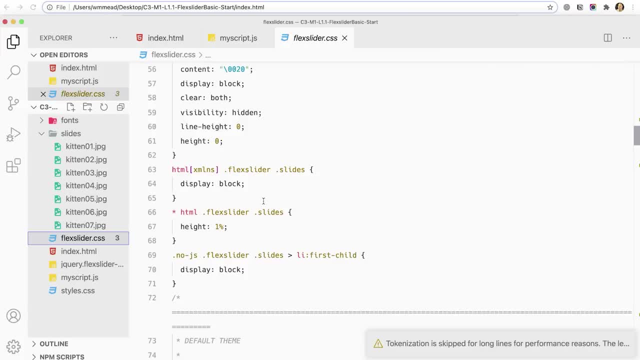 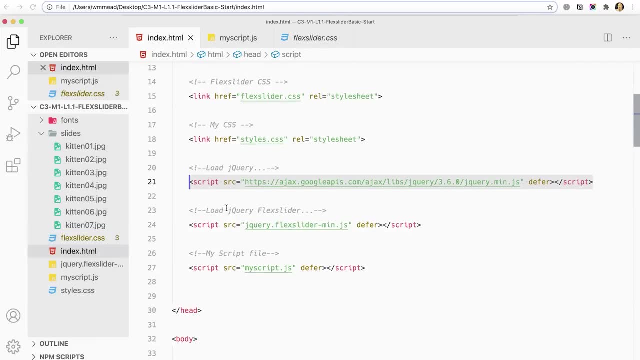 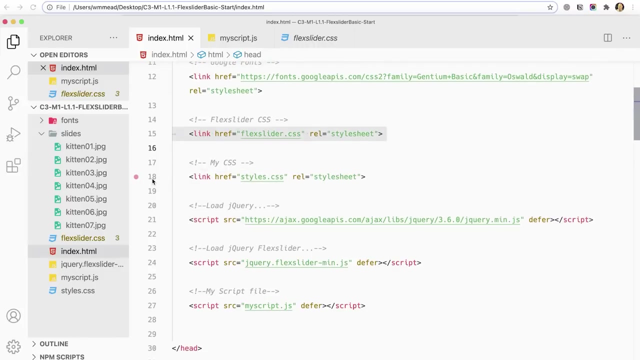 update this slider script to a newer version. i don't want to lose any changes that i've made. so this is one of the main reasons why i want to make sure that my script, my css file, loads after their css file, because if i can add a rule on my css file, 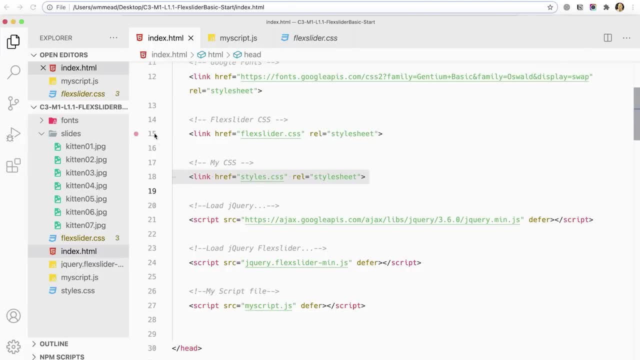 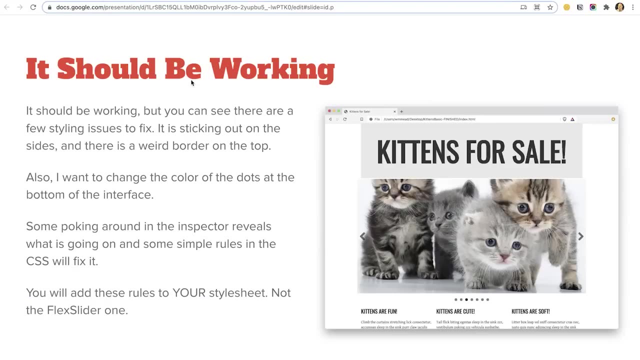 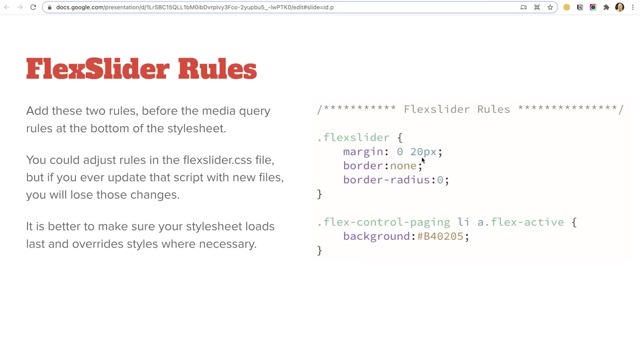 that says dot flex slider, then i can override the rule over here. so what do i want to do over there? to do that, i want a rule for dot flex slider. i want to set the margin to this zero: 20 pixels. so zero on the top and bottom, 20 pixels on the left, right border, none, border radius, zero, and that will clear out. 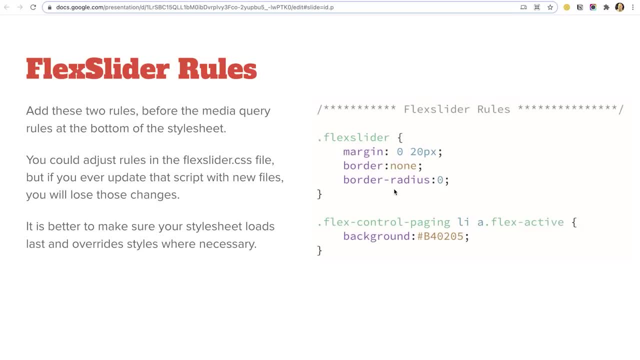 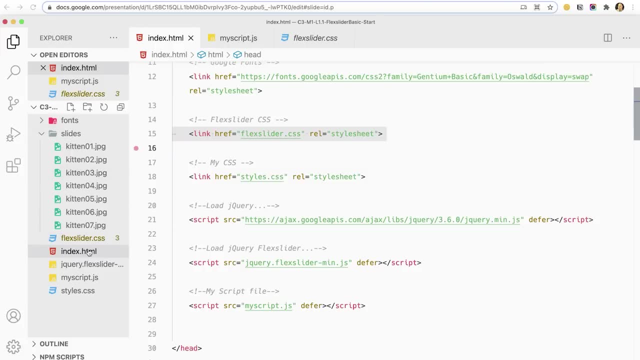 some of those styles and kind of clean up the styling of the actual flex slider. so let's go ahead and add that to ours. and how do i know that? just by poking around in their css file. so i want to make sure i'm on my css file, which is where 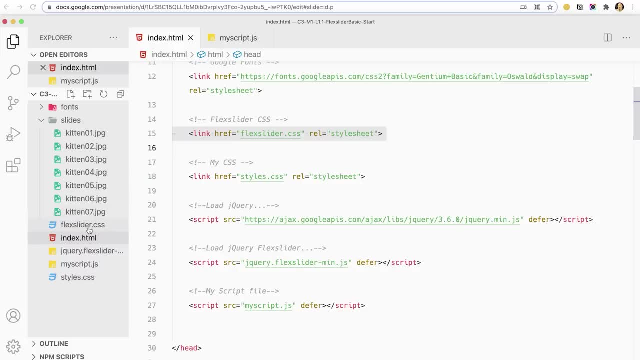 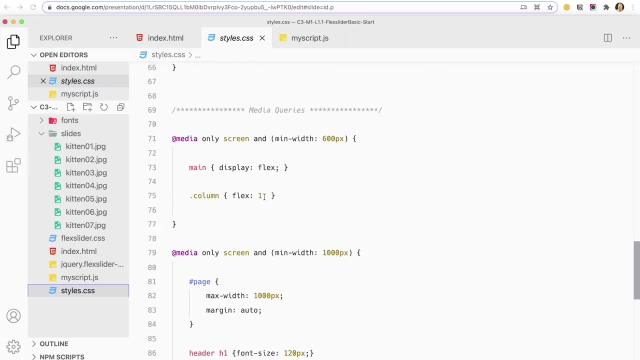 i don't want to do flex slider css, turn that one off, stylescss. there we go, and then somewhere in here you can put it wherever you want. it doesn't really matter. make sure it goes above the media queries. maybe i'm going to make a comment here that says: 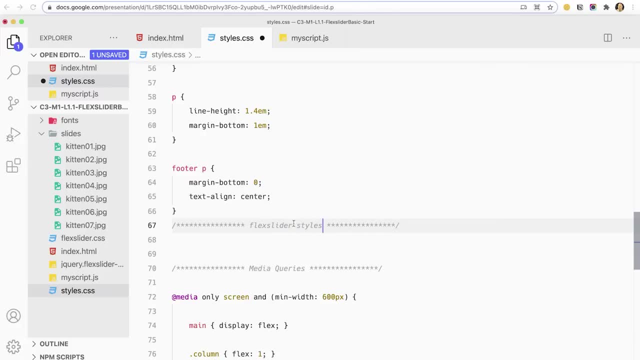 flex slider styles, and in here i can make a rule dot flex slider margin. i wanted zero on the top and bottom and 20 pixels on the left and right. i want border none, no border at all, and border radius zero. give it square edges. just with that one rule in place here, with that one rule. 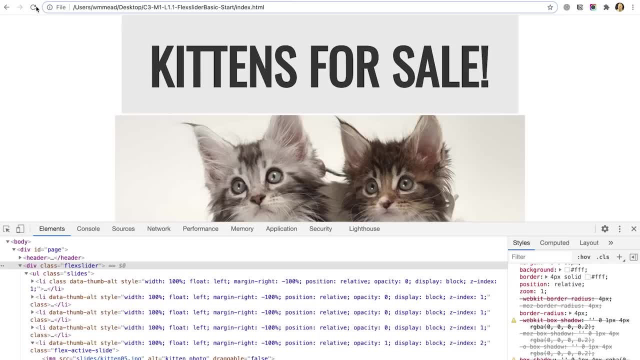 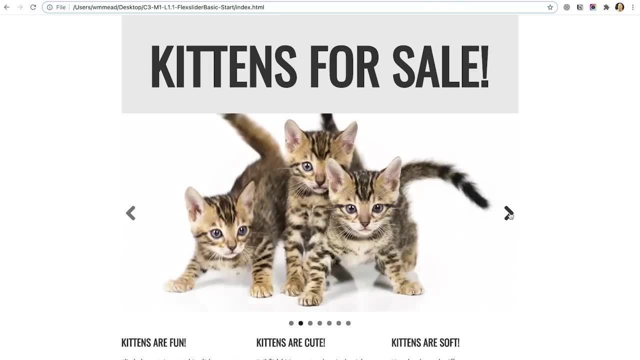 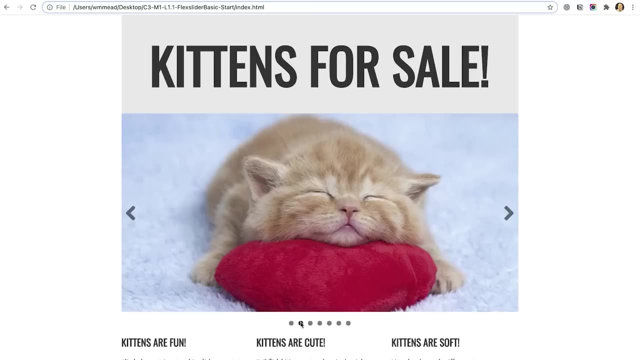 if i come back and check my page, you'll notice that the flex slider looks better here. it's fitting into the space well and i've got gotten rid of that gap and all that kind of stuff down here. i still want to adjust these buttons a little bit, so i'm going to inspect again. 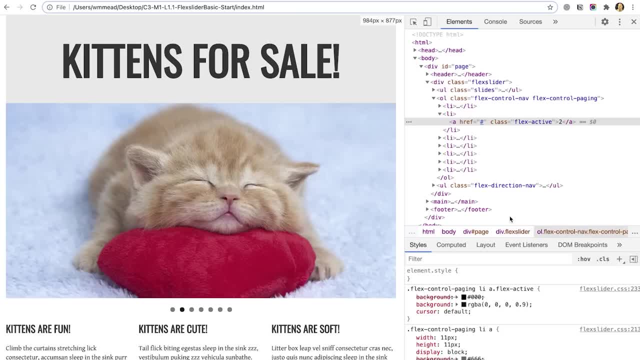 maybe move my inspector to the side- and it's this thing here: dot, flex control, paging, li a flex active. that's the class that's creating, that's changing the colors on these buttons here. so that's the one that i want to actually attach to. so i'm going to come over here, i'm going to 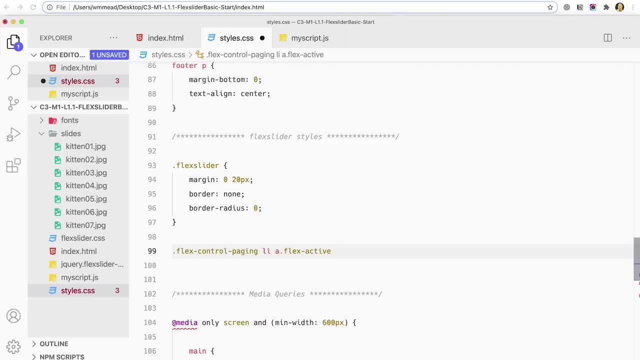 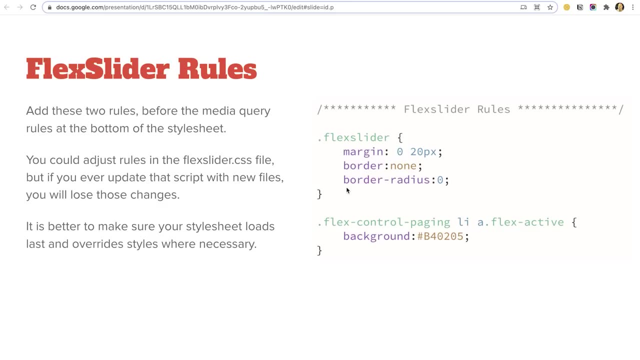 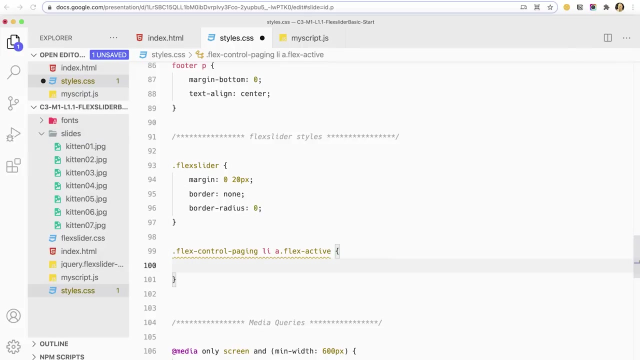 add that rule in here if i want a different color. what did i put on my slides over here? i put pound b40205. make it match that. what was it? just color or was it background? background would be pound b40205, and what was it? 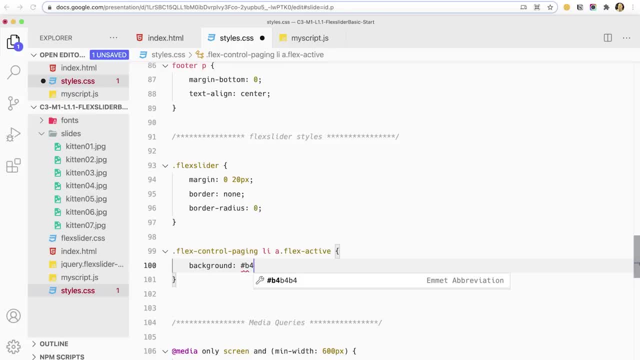 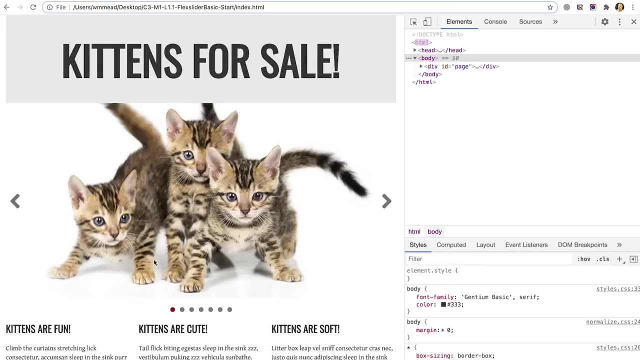 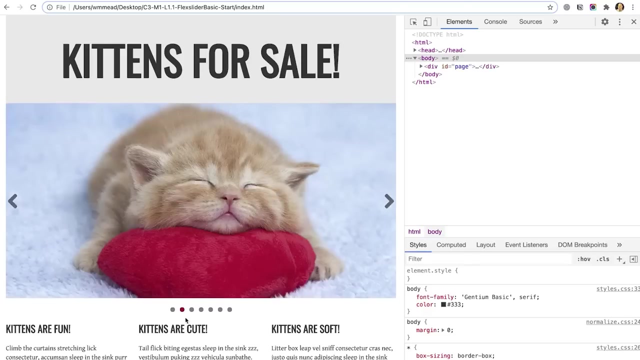 and what was it pound? i've forgotten already. 402, 205, there we go, and that will give me sort of a red background color. save that and come back and test it and you can see my color is now overriding the color that was there before, and I can go ahead. 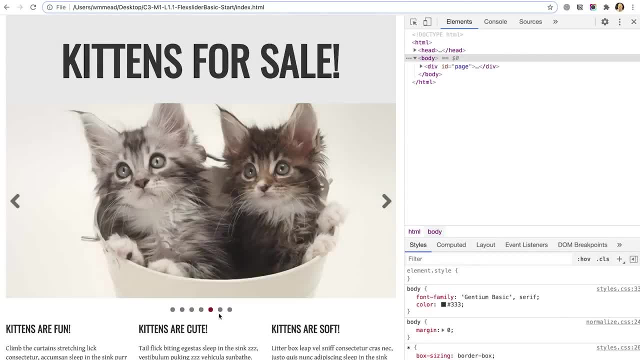 and click on these things and they all work, so that's great. so you want to put styling on your own style sheet that will override styles on the flex slider css to customize it to make it look the way you want it to look, and finding out what those styles are are just a matter of using the. 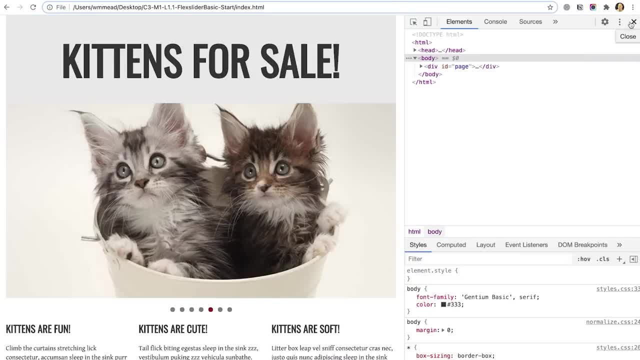 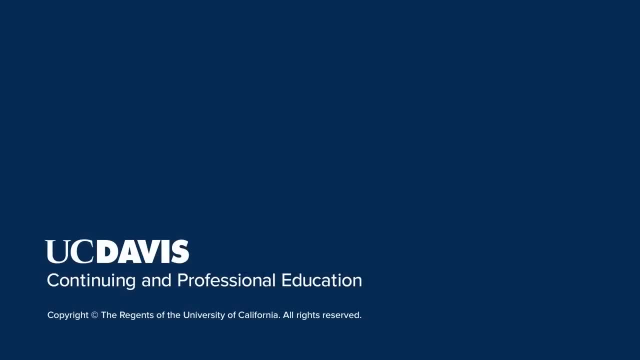 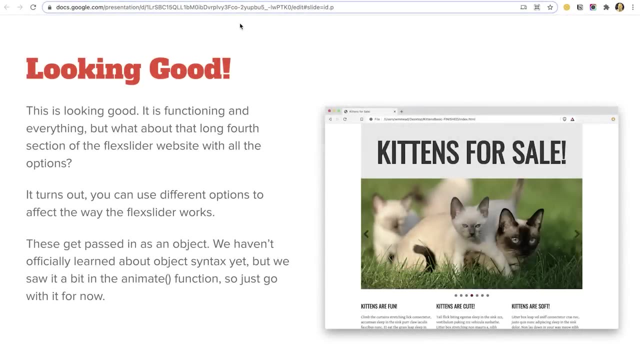 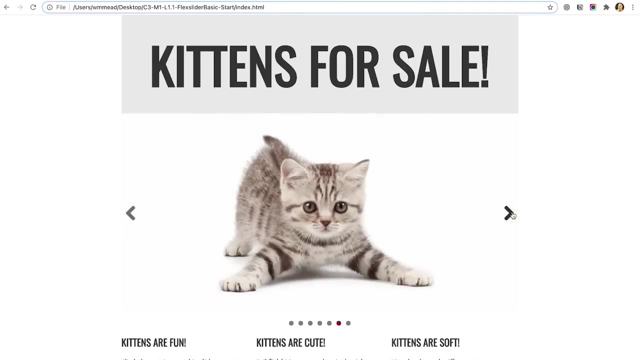 inspector and hunting around to see what rules are being applied that you might want to change to get it to style and look the way you want it to look on your page. your slider should be looking good. we've gotten everything in place and it's working. it's functional and it looks good, and we've adjusted the css. 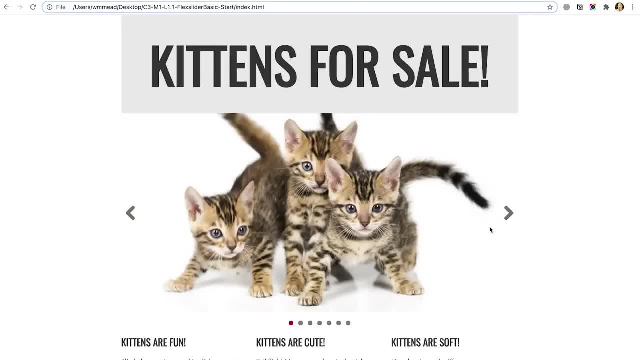 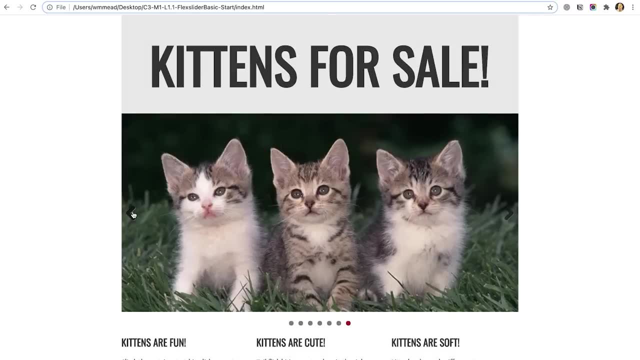 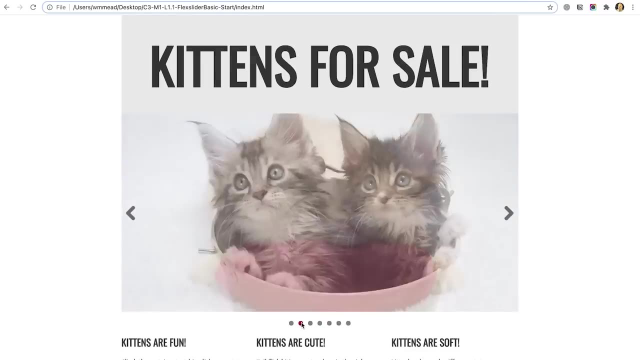 and all that kind of fun stuff. so that's really great, and it's a lot easier to do this with just a few lines of code than having to write all of this functionality ourselves, especially since you've seen how to make a slider. we didn't include this functionality for being able to. 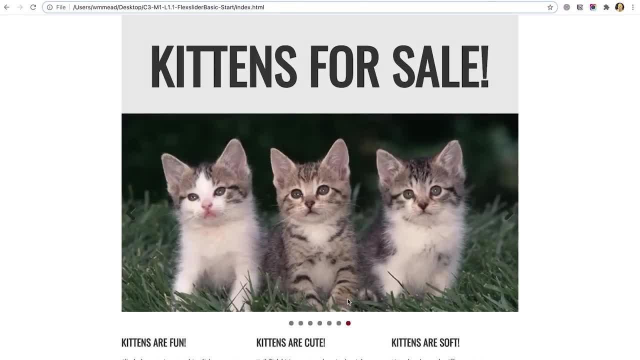 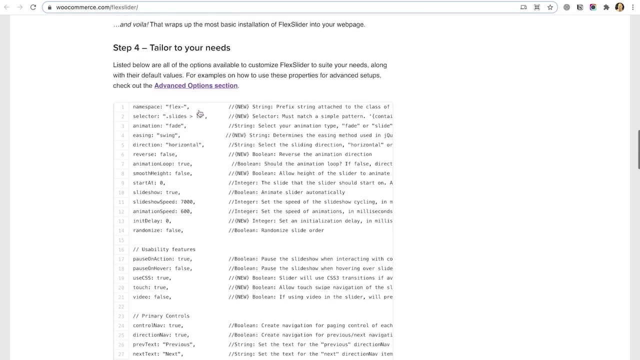 have these buttons down here, being able to go to slides that way, but we could have done that manually on our own, but with this plugin it provides it for us automatically, and that's great. now what about all these additional options that show up down here at the bottom of the screen? there's all this stuff down here and we can use this to further. 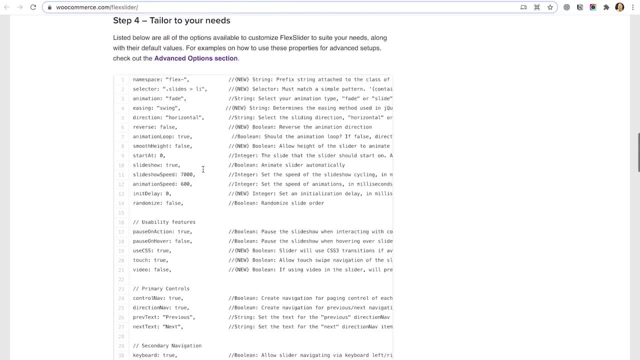 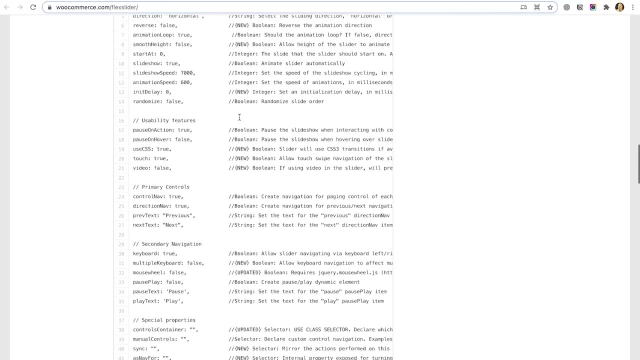 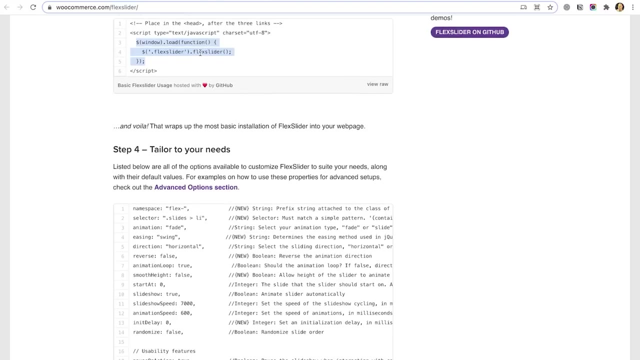 customize the functionality of our flex slider, and that's really cool. but how do you do it? it's not really clear, by looking at this, exactly what you need to do. but basically, what we need to do is we need to pass options in to our flex slider and we need to pass options in to our 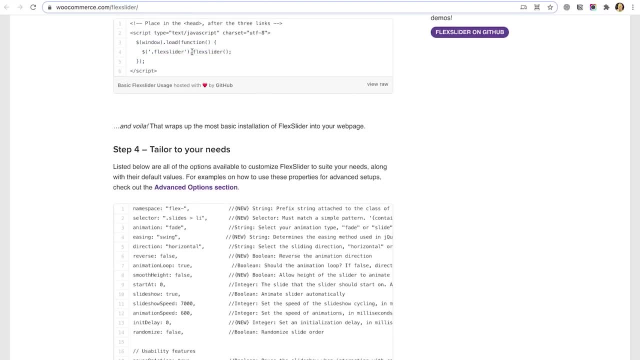 this flex slider method here, this flex slider method here, and we pass them in in the form of an object, because these things here are look like key value pairs that you can pass into an object, and it would be really nice if they made it really clear on exactly how to do this. 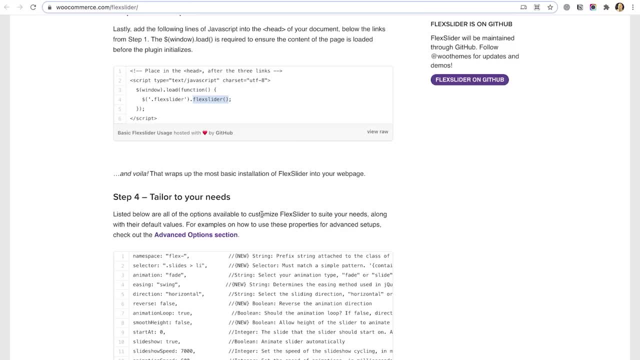 here on the instructions. but if you know some javascript and you're familiar with having done this kind of thing before you figure out how to do this, and you're familiar with how to do this- you can figure it out pretty quickly. so what can we do? let's take a look at it. 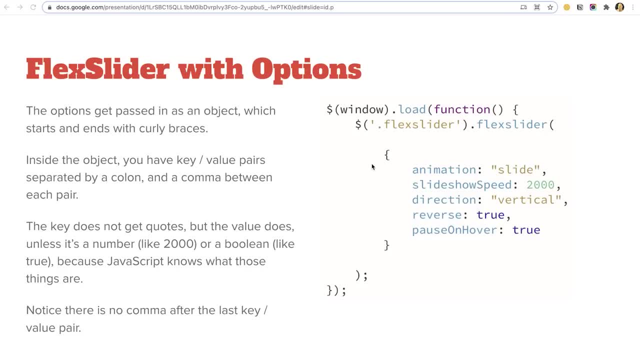 just like we did with the end, with the custom animate method in jquery, we can pass in an object- curly brace, curly brace, and then we can pass in these key value pairs to get the slider to do some different things. so, um, let's give that a try, and i know we haven't really talked a lot about objects. 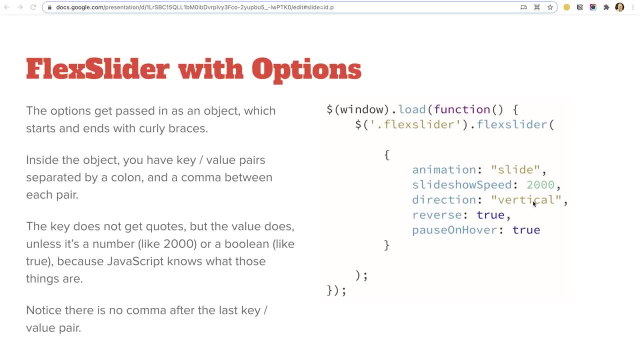 yet and we will get into that in a little bit. but let's give that a try and i know we haven't really talked a lot about objects yet and we will get into that in more depth in a in a lesson coming up, but for right now we'll just kind of go with it. 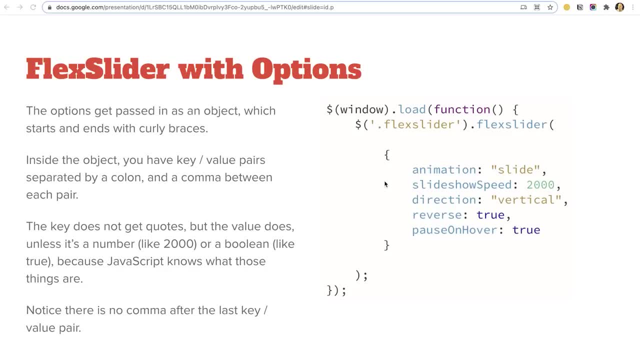 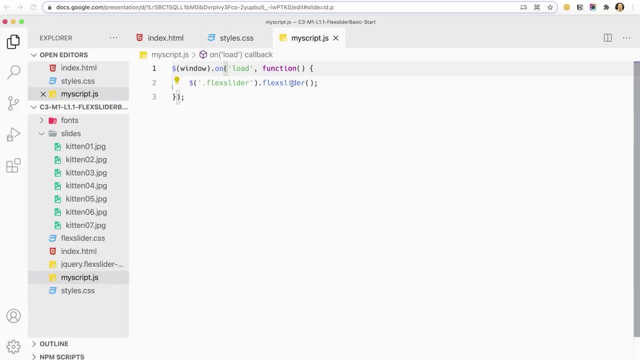 and get used to this syntax, because we'll see it a lot, especially with plugins. so let's come over here and inside our script file, here, inside our parentheses, here we're going to add a set of curly braces and then inside these curly braces we can add different settings. and what are the? 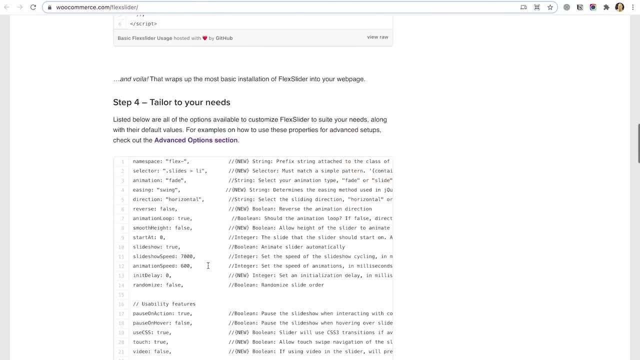 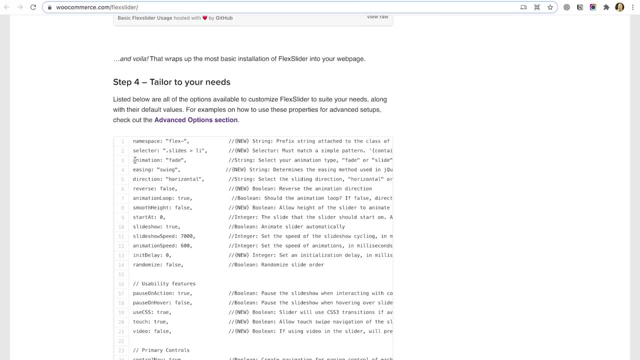 the settings that we can add. well, there are these settings over here. so, for example, if you wanted to do animation slide, so you can. you can set it your feet, set your animation to fade or slide. by default it's doing fade. so, over here, when we go from slide to slide, it's fading. from slide to slide, it's doing a. 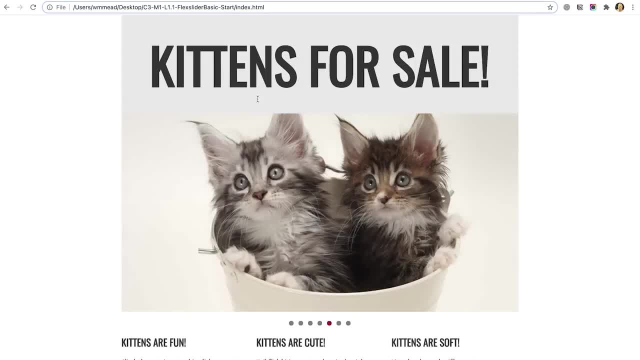 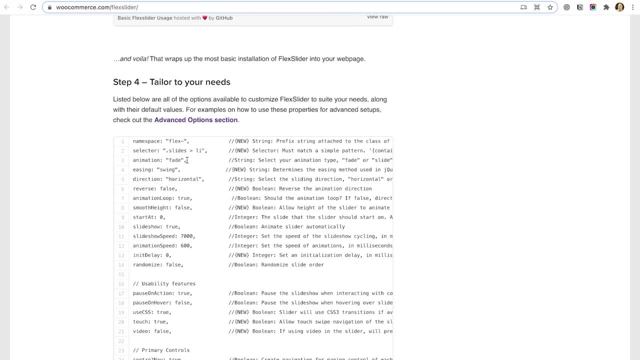 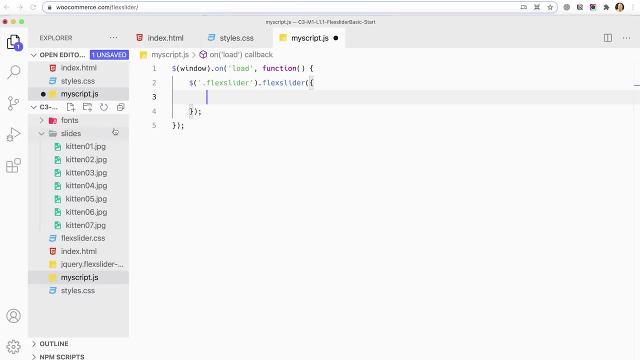 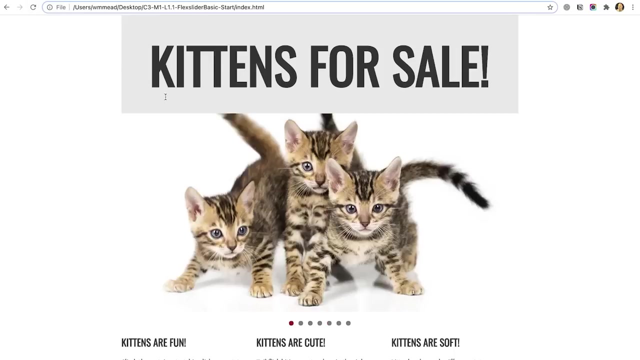 fade in, fade out, but if we wanted to actually do a slide, we can change that to animation slide, so you could take this, copy it and then come over to your script and stick this in here and change this to slide. get rid of the comma, because if I do that, you'll notice over here immediately: refresh when I click on. 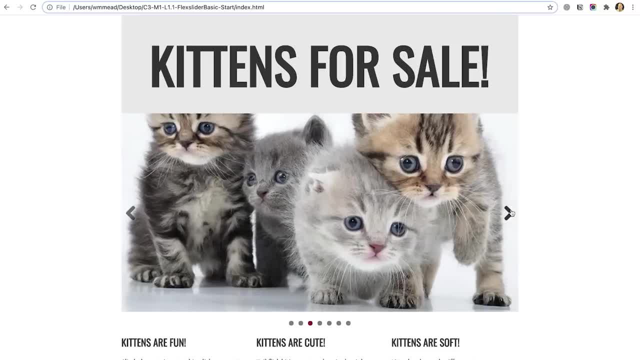 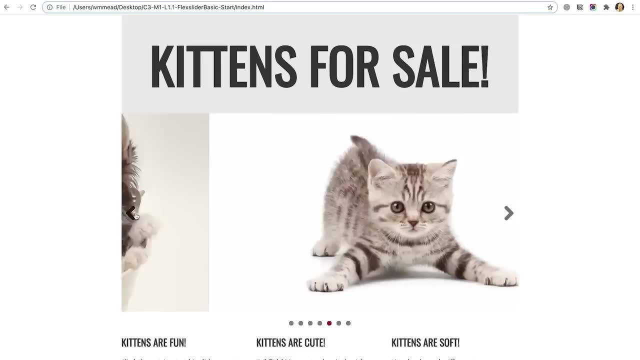 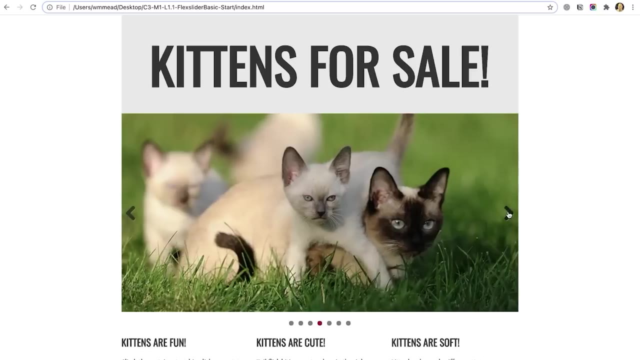 the next thing: instead of fading, it's sliding. and look at that, it loops around. don't have to do any special programming for that, it's all built right into the plugin and you remember what a trouble that was for us to figure out how to do manually. well, 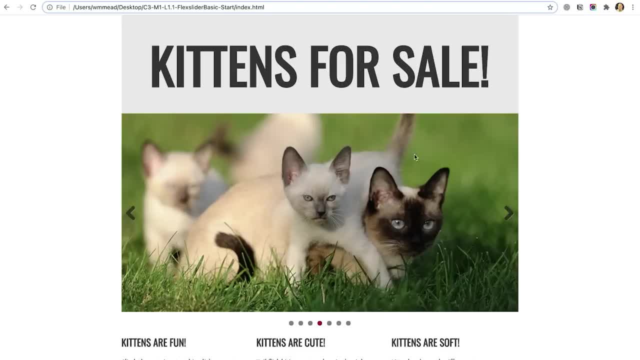 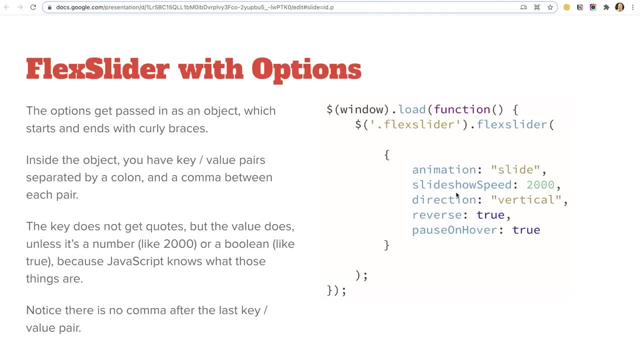 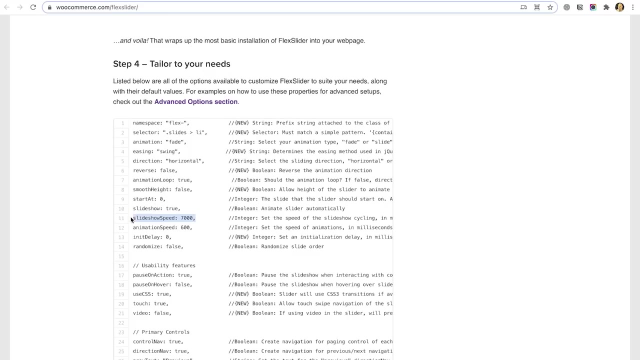 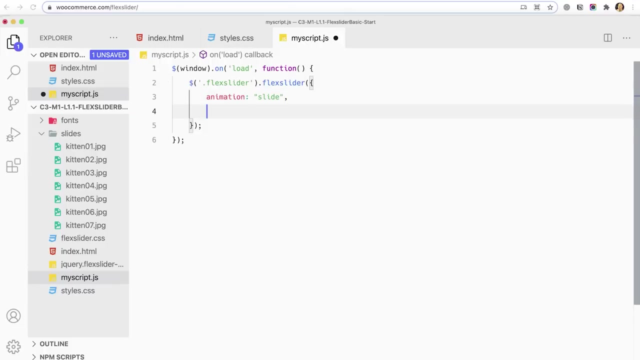 here. it's built in so we don't have to really even worry about that. what else could we do over here? I had slide, I have. you could set the speed- slideshow speed that's in here. slideshow speed, slide comma. for each one of these in here you have to put a comma at the end, except for the last one, I'm. 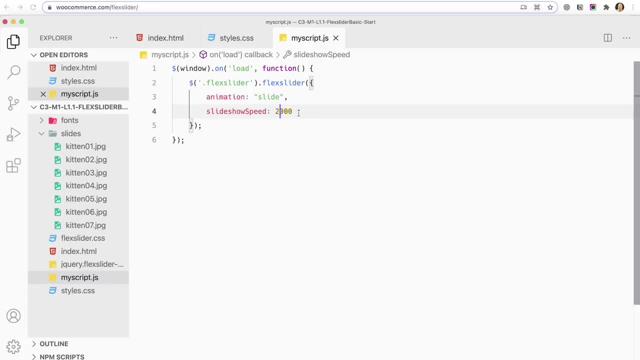 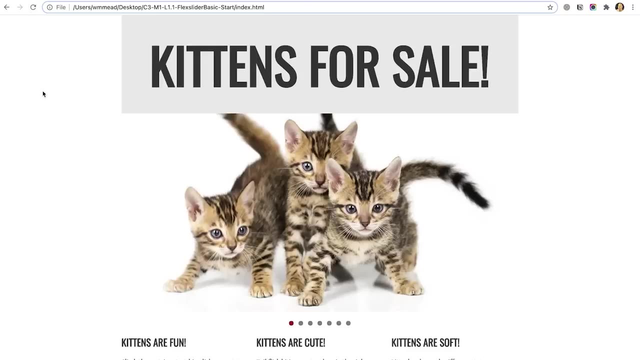 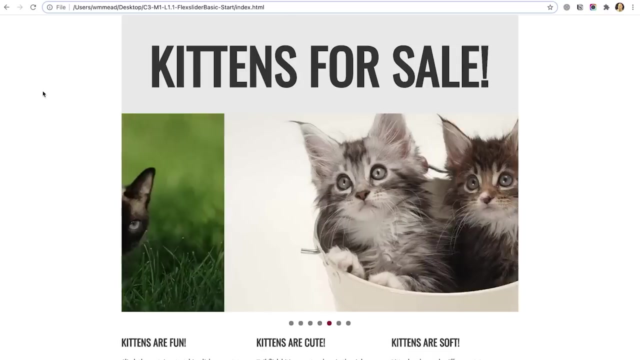 not going to set it to seven seconds, that would be really long. I'm going to set it to two seconds. that will tell us how quickly it's gonna slide from slide to slide automatically quickly. One, two, One, two, There we go. So now it's going rather quickly, So that's. 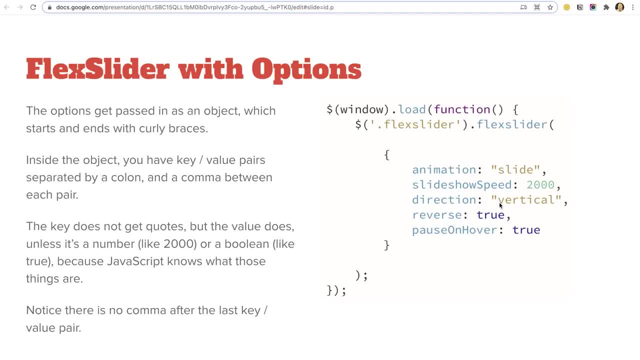 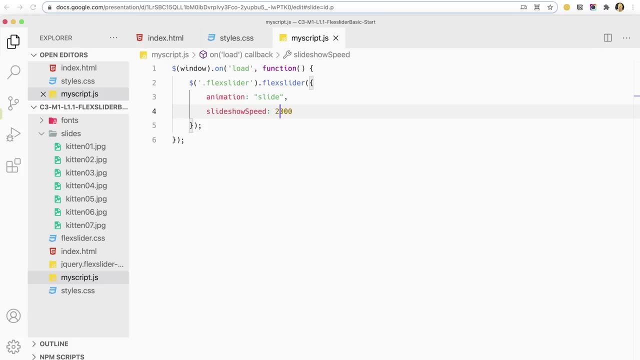 great. What else could we do? We could do direction vertical. If you wanted to just slide up and down, instead, we could do that Comma: direction vertical. This has to go in quotes because it's a word that JavaScript doesn't know, but it knows that one there. 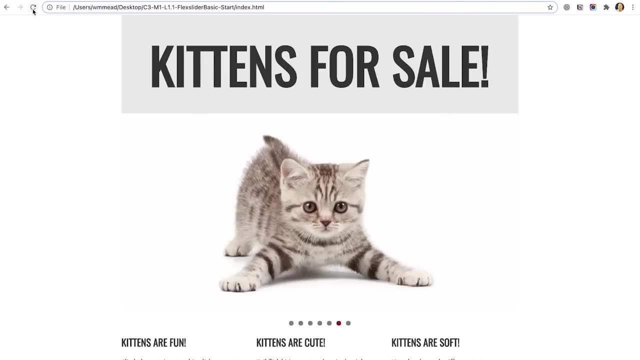 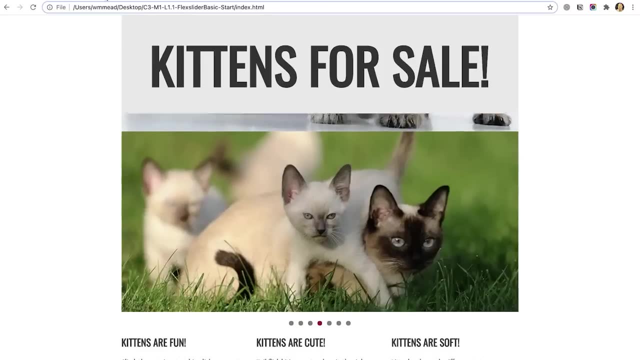 It knows what 2,000 is All right. so now, if we do this, after two seconds, it's going to go vertical. We could do reverse, true? so it'll go from top to bottom instead of from bottom to top. 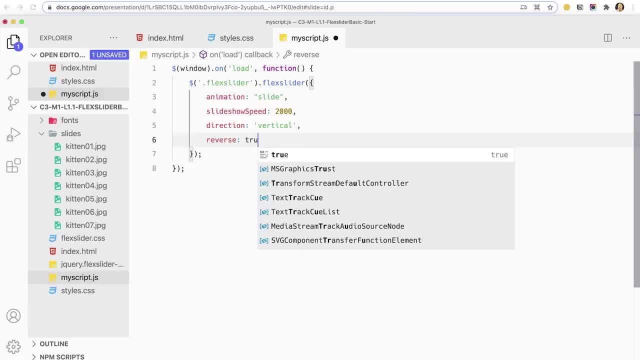 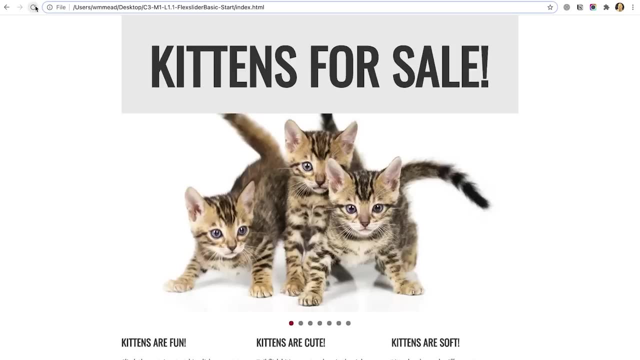 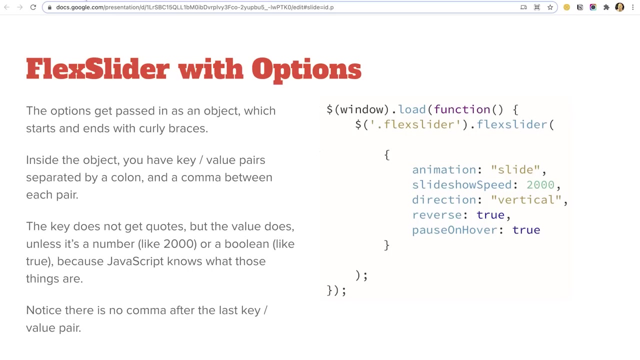 Reverse true. True is a word that JavaScript knows. Now it's going from the top to the bottom. And then, finally, another one we could do is pause on hover true, which is in here. You can find it in here somewhere. pause on. 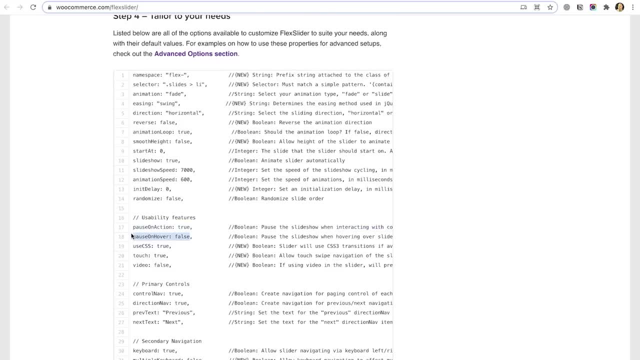 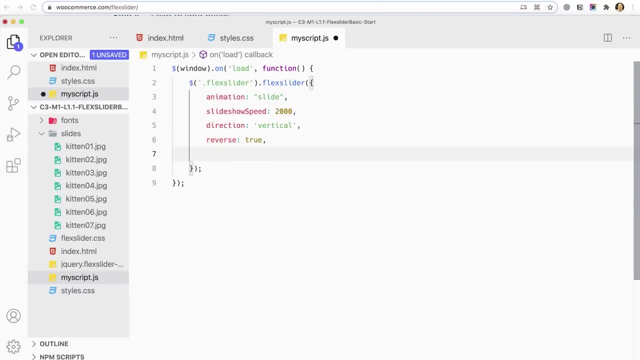 hover. There it is, So we had set this. This was a feature that we had tried to build into our own version, that we did build into our own version. Set that to true, And when you're hovering over the slides, they'll stop. It's a very nice interface, And then we could do. 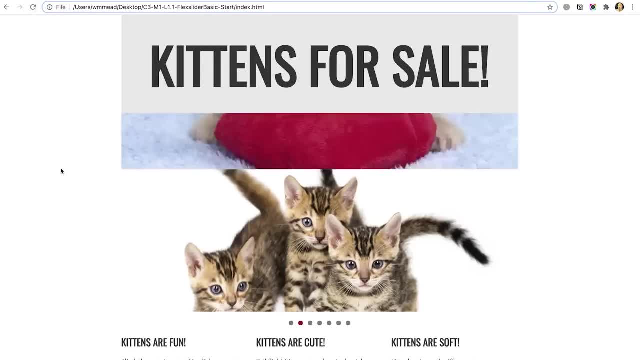 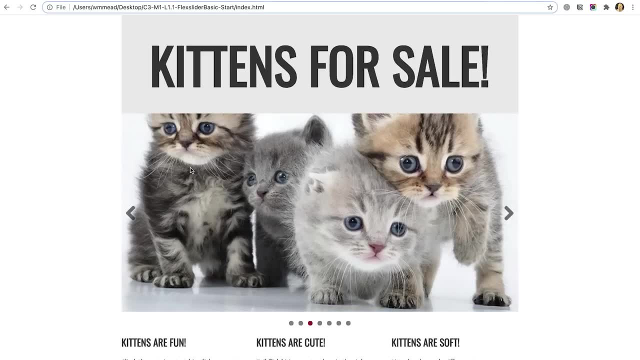 the same thing with the other interface element, right. So now, every two seconds it's going to go, unless I hover over the slides, in which case it's going to stop And it won't. Because I want to enjoy these kittens, I want to look at them for a while. Two seconds isn't really long enough. 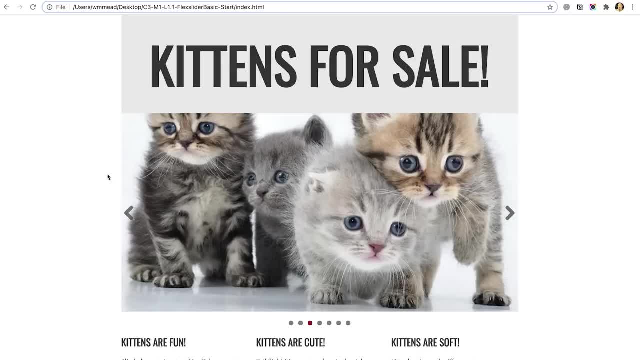 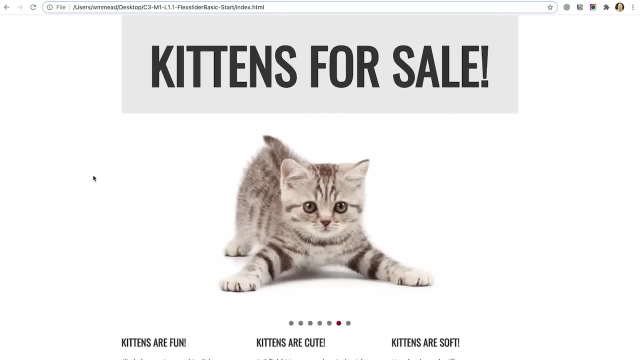 So I can really enjoy them and look at them for as long as I want, And then, when I stop hovering on it, it'll wait two seconds and it'll start going again. So that functionality is built in as well. So that's great. 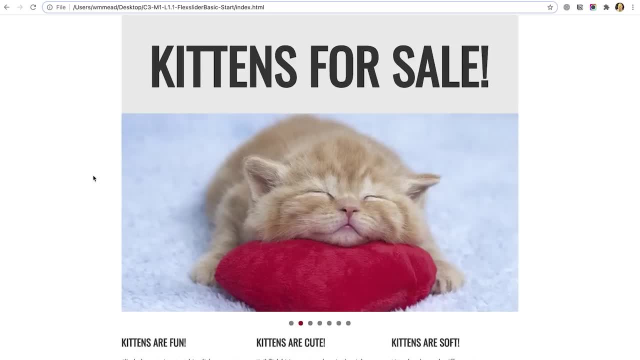 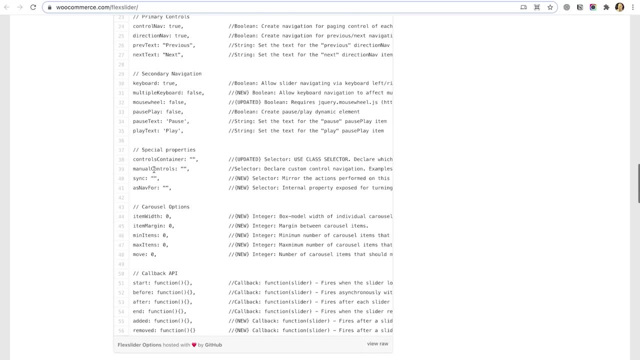 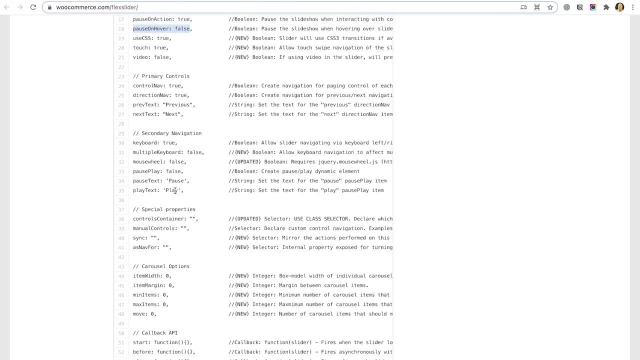 It gives us a lot of opportunity to build in a lot of extra functionality. through these additional features that are here- And there's a lot of them- Manual controls, controls, container- you can do all kinds of things. Those arrows: you could swap those arrows out for something else. 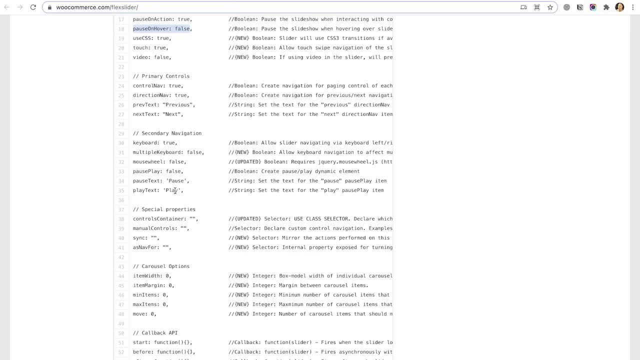 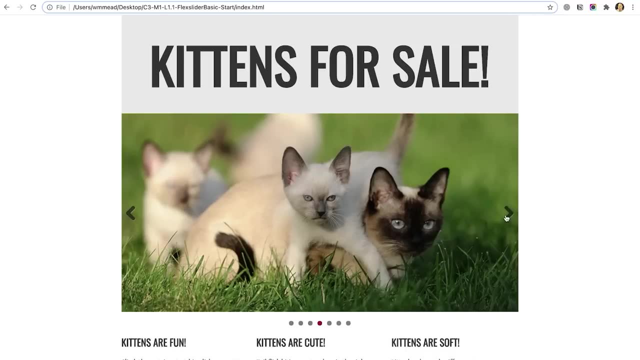 so that it doesn't look like every website you go to that has Flex Slider on. it could look the same, because they all have the same arrows here- left and right arrows- But we can get rid of those and do something else. That would be kind of interesting and fun. 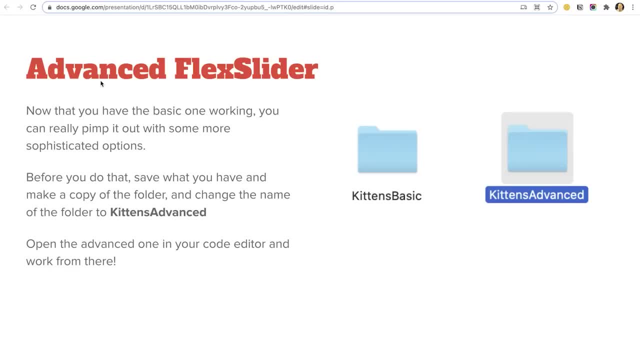 Now that you've created the basic Flex Slider with some advanced options, we can really do some different things with this Flex Slider, And to do that, it's kind of nice to keep the basic version working the way it is working, so that you have a version of that if you want to refer back to it. 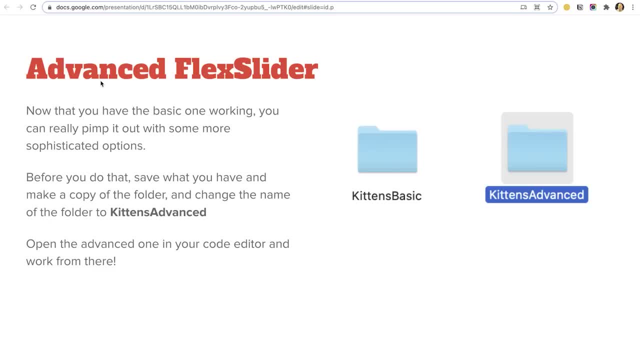 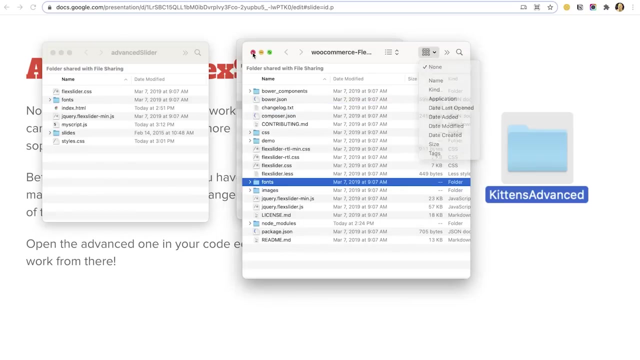 So if you want to, you can duplicate that folder and create a new folder and change the name to something like Kittens Advanced or something like that. You can see over here. I have actually changed mine here, So I don't need that folder anymore. I can close that one, But I just duplicated. 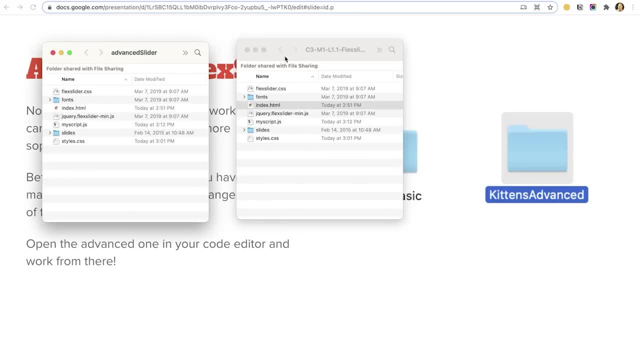 and called it Advanced Slider. So this set of files is currently exactly the same as that set of files, but I've made a copy so that I have this version. I want to refer back to it, but I'm essentially done with it And now I'm only going to work on the 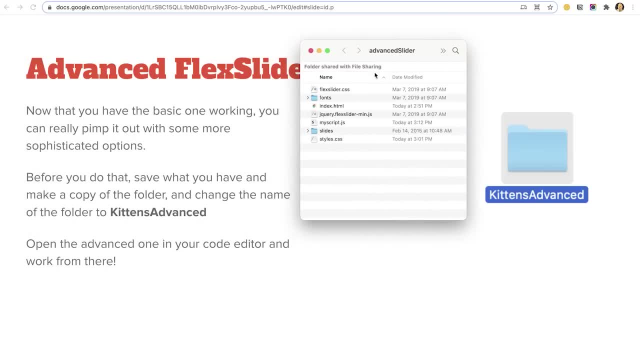 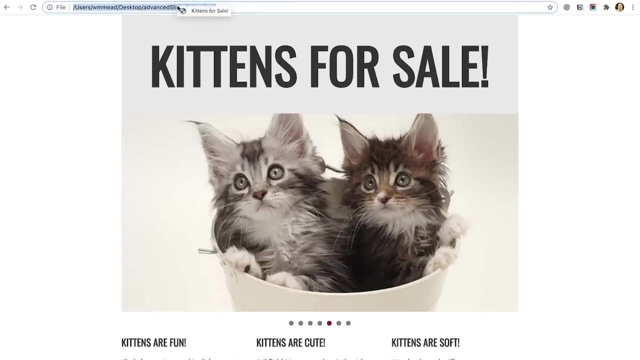 Advanced Slider version here And I have that version. these files open in my code editor and I've also switched this over here so that it's pointing to my Advanced Slider folder here, so that I know that I'm working with the right set of files. 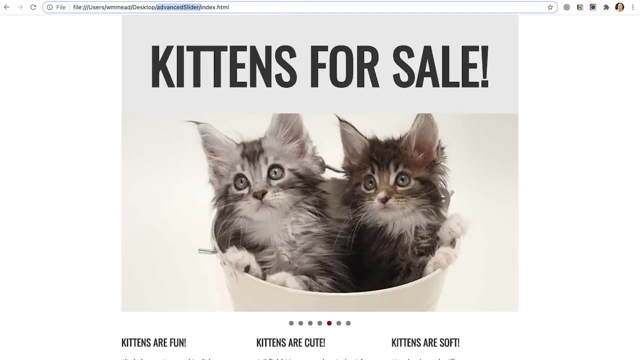 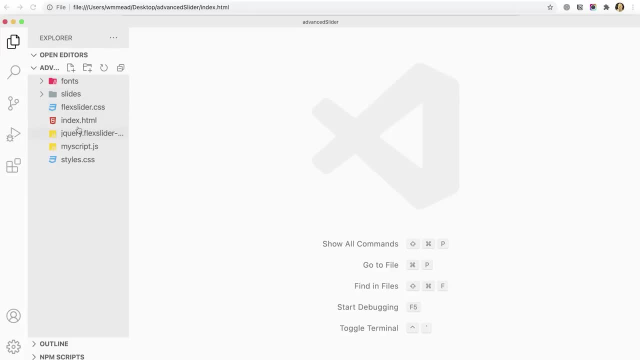 Okay. so make sure you're working with the right set of files in your browser. Make sure you've got the right set of files in your code editor Over here. you can see it says Advanced Slider there. So this is my Advanced Slider files. 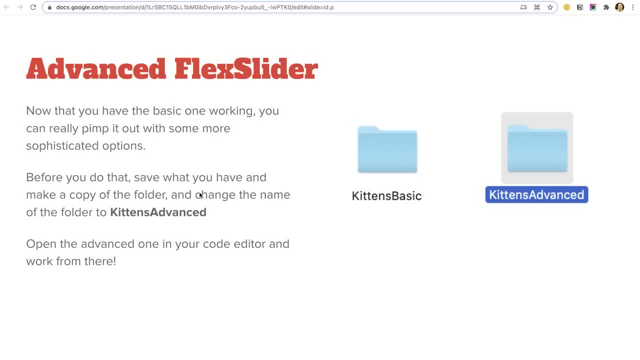 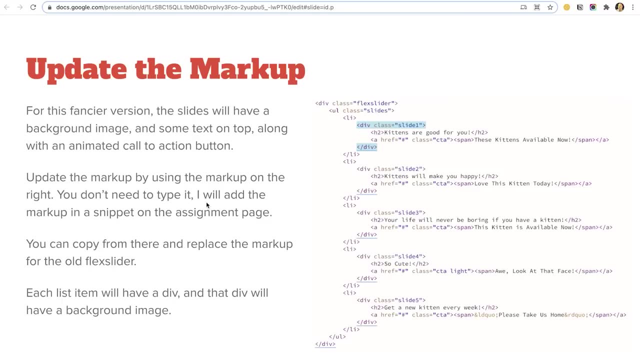 Alright, great. So now that I've got that into place and I'm ready to really do some different things with this Flex Slider, the first thing I want to do is I want to have a fancier version where I actually have some content on top of each slide. 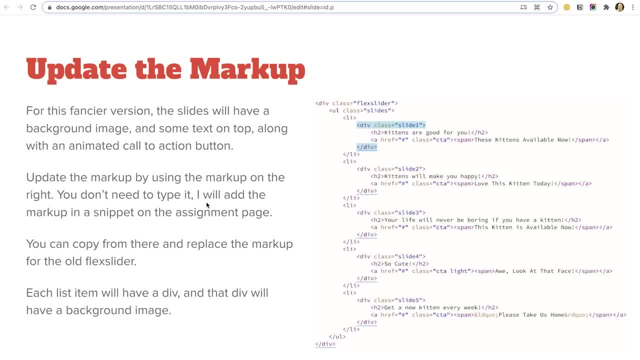 like we did with the JavaScript version of the slider, where we had a div on top with the heading and a paragraph and then the slides. the actual pictures were background images on the slides And I'm also going to have an animated call-to-action button that will drop down and make it really clear. 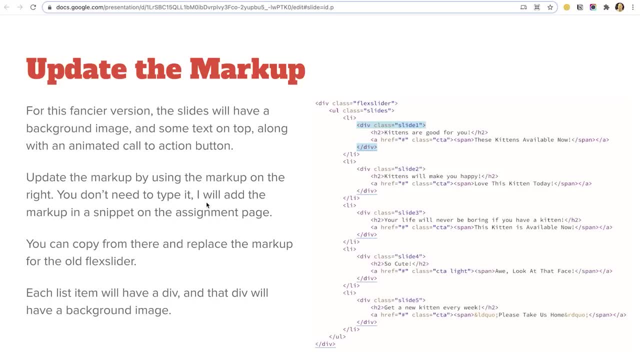 that what you should do is adopt one of these kittens on this lovely kitten page. So I need to update the markup to go along with this for my Flex Slider, and I will provide some snippets with this link, So I have this lesson that you can open, and they look like this: 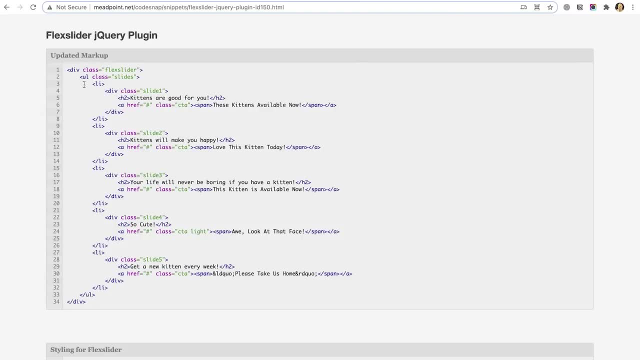 There's some snippets here, And so I'm basically going to replace my slider with this content here. You could type it all out if you wanted to, Instead of just putting the pictures in. I have a div with an h2.. The div has a class of slide1,, slide2, slide3, so on and so forth. 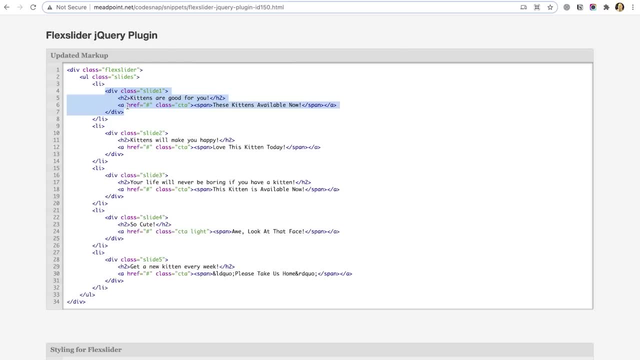 And then I have the h1 and the h2, and I have an anchor tag with a class of CTA for call-to-action and a span around the text- which I'll explain what that's going to do in a few minutes- that says these kittens are available now. 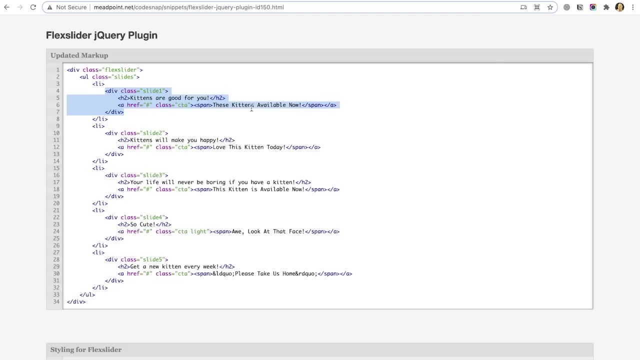 So this is going to be like a call-to-action button that you can click on to access these kittens, And it's not really going anywhere because the link is just set to a pound sign, but if this was a real website, that could be a link to a page. 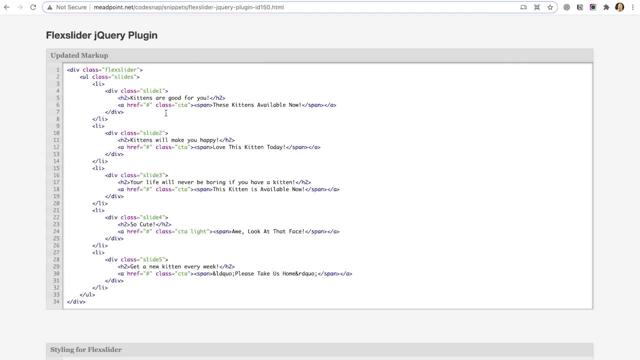 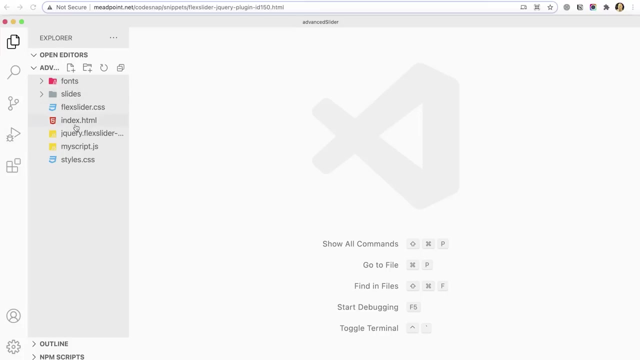 where you could actually adopt this kitten or something like that. That would be kind of fun. But rather than make you type all of this stuff out, which is kind of tedious, you can actually come to the snippet page and just copy it and then come back to your project and on your index file. 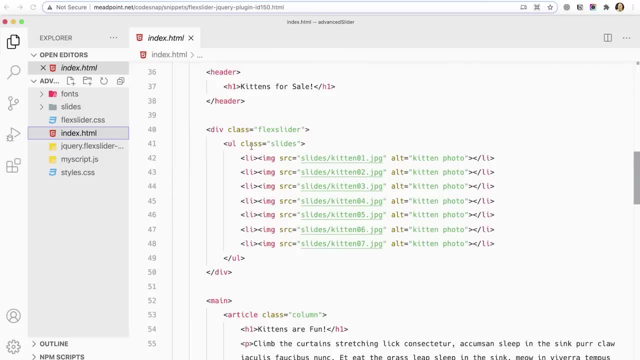 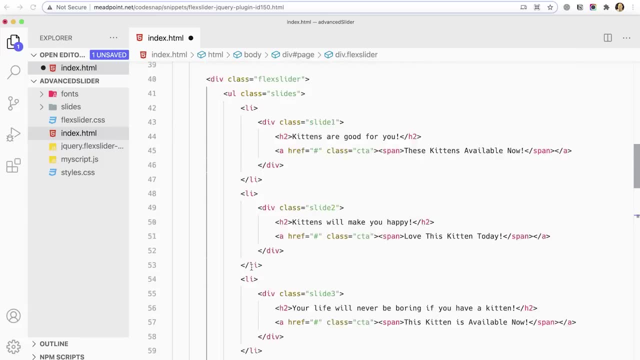 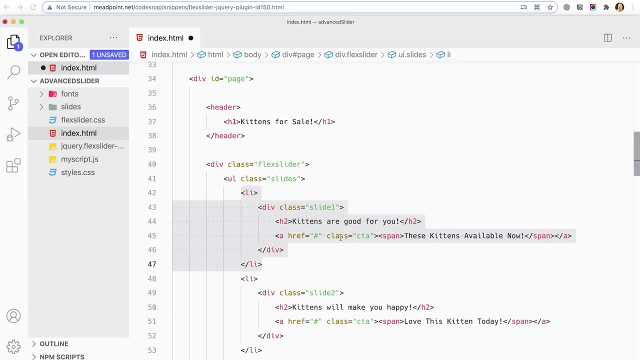 in place of the slider down here, this flex slider. we're just going to paste this one in instead. Paste that in, And it's still div class flex slider, still ul class slides. All that's changed is that The list items in here. 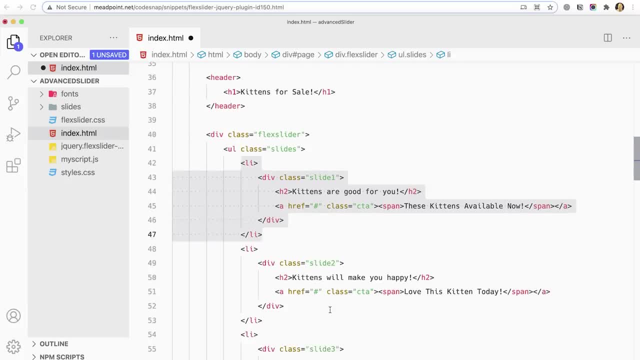 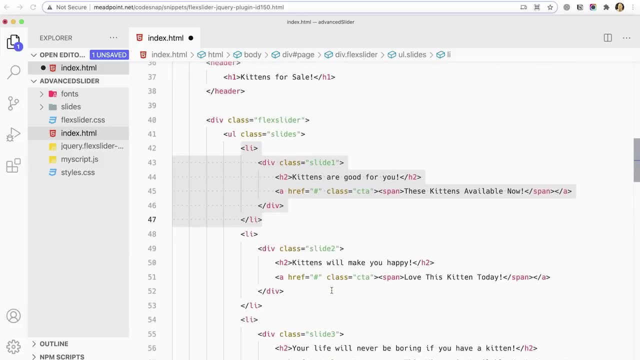 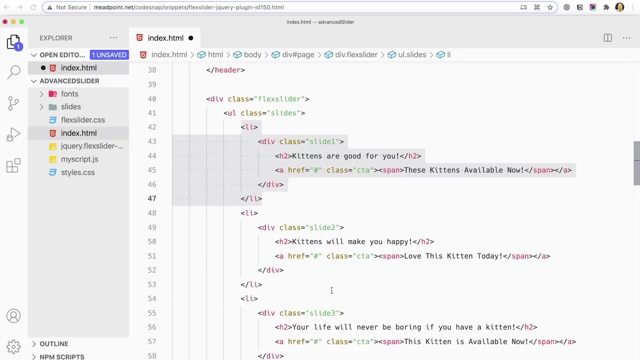 These divs have a class of slide one, slide two, slide three, slide four and slide five. I dumped slide six and seven for now. Probably five kittens is enough for this slider And that's great. Okay, So that gets us started, and on our way, with creating our fancier version of our flex slider. 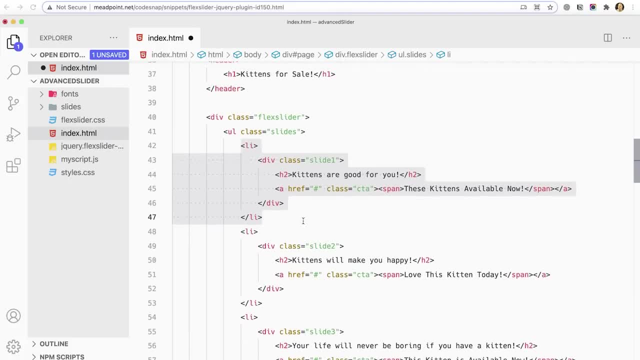 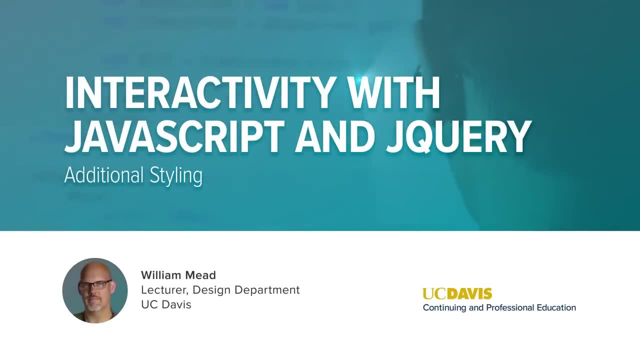 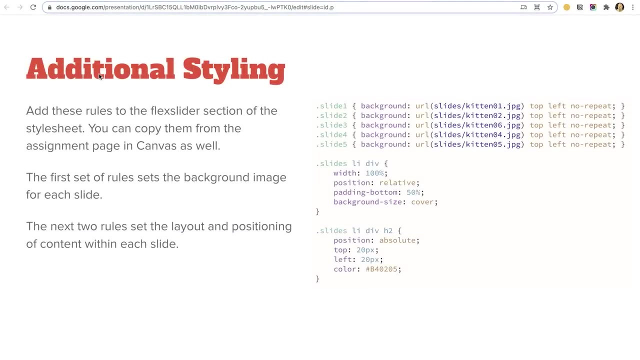 In the next video we'll start looking at what we need to do to adjust the styling for this. In the last video we updated the markup for our fancy version of the slider And now we need to do some updating for the actual CSS for the display of the slides. 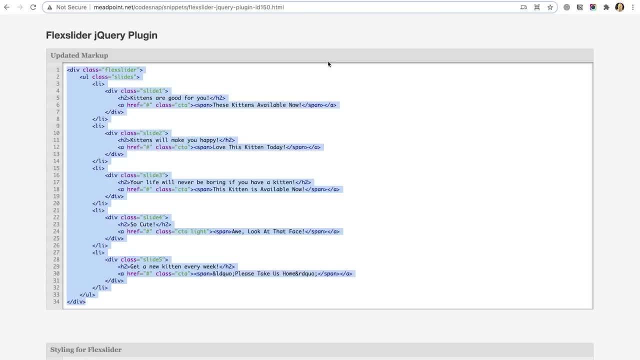 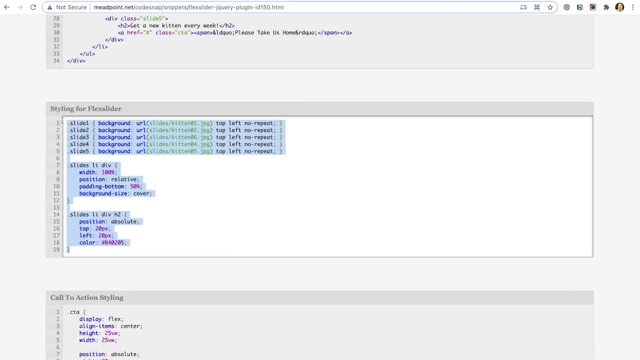 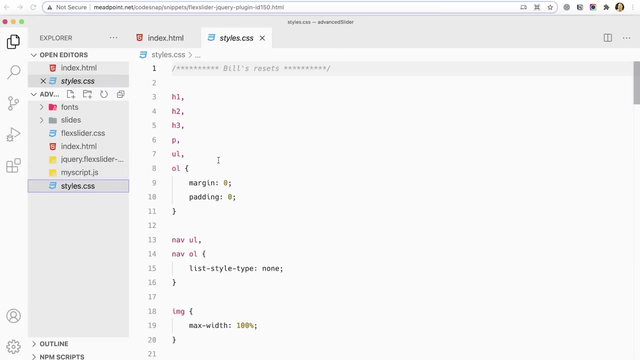 So I'm going to come back over here to my snippets And I'm just going to copy these, these three rules here, And I'm going to come over and paste them into my CSS file Style over here, StylesCSS, And I'm going to stick them just in my section with the flex slider stuff here. 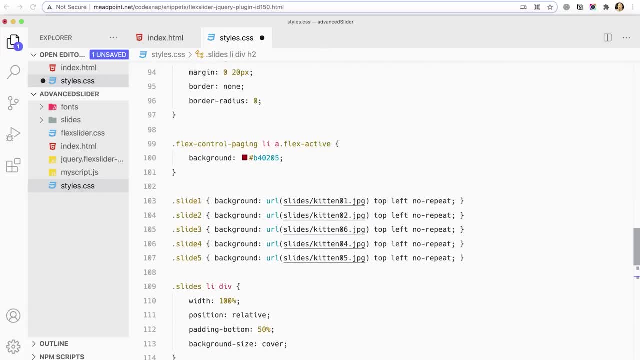 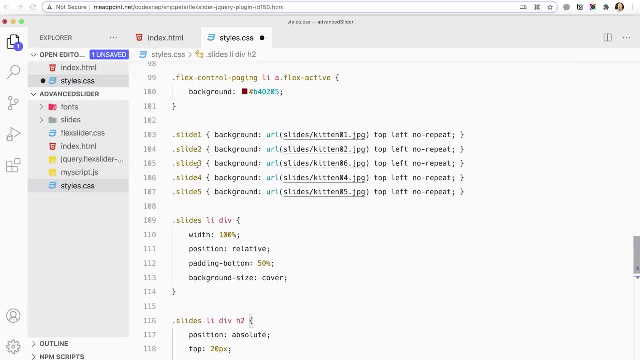 It doesn't really matter where they go, I'm going to put them here Now. this is really important. The slides: the dot slide one, dot slide two. dot slide three, that corresponds to these divs, Div class. slide three. slide four: 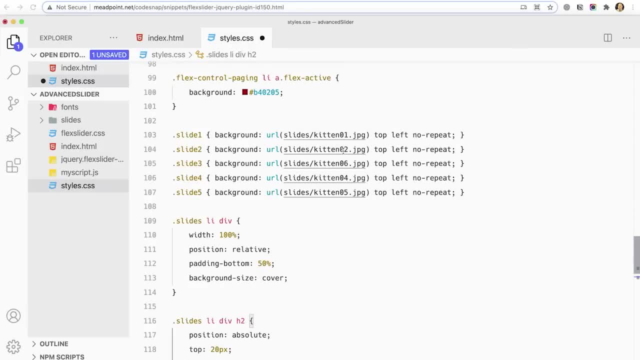 They're going to get a background image. Each one is going to get a different background image. The background image is positioned at the top left and said not to repeat. Now, one thing that's important about this particular slider that you have to remember is that it's flexible. 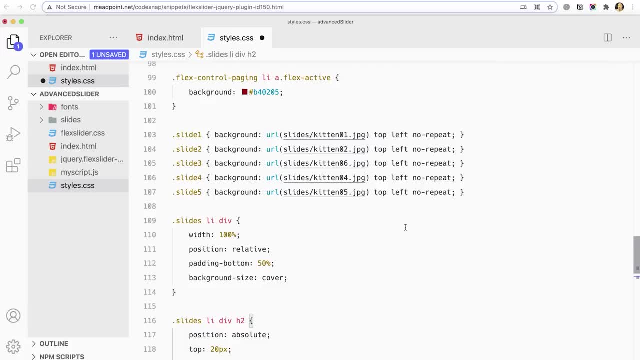 That's why it's called flex slider, And it'll work for responsive websites, And you can make these slides bigger or smaller. So we have to pay attention to the proportions of the slides, from their horizontal width to their vertical height. What is the proportion there? 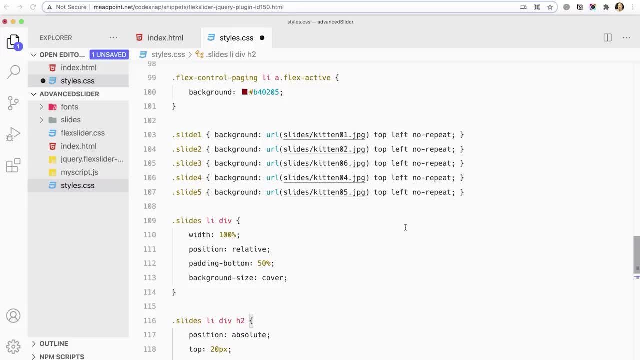 We want to keep the slides in proportion so that if they resize on the screen they resize proportionally, And keeping track of proportions is a little bit tricky in CSS currently. There's some features coming to CSS that will make it easier in the long run. 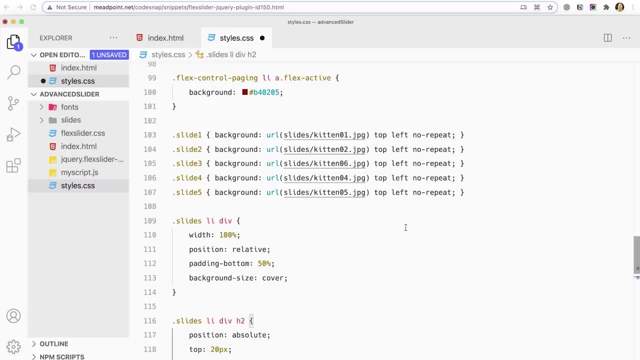 But for right now it's a little kludgy and unfortunate. But basically what I've done here is, I've said, the div that's inside these list items, I'm going to make it a width 100%. I'm going to make it relative because I'm going to absolutely position some stuff inside of it. 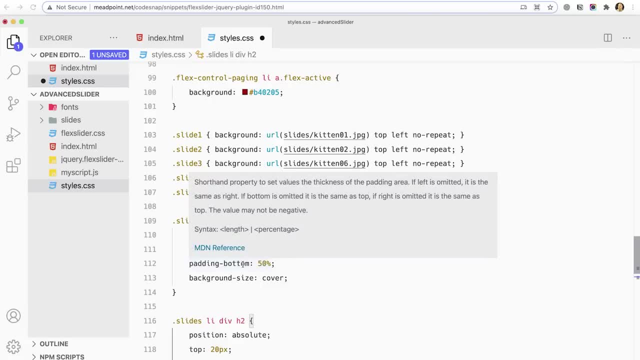 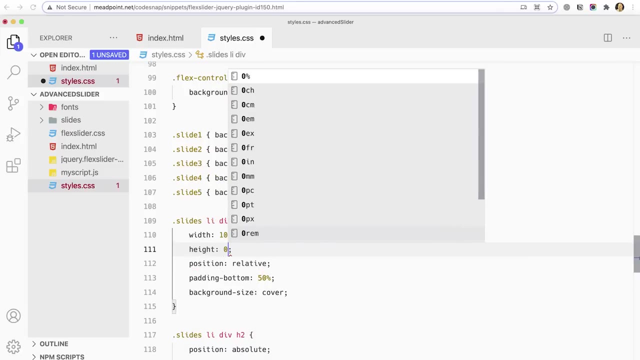 And I set the padding on the bottom to 50% And it could be either padding top or padding bottom And background size cover And essentially the height of these, and I probably should add in here height 0.. Height 0.. Add that in as well. 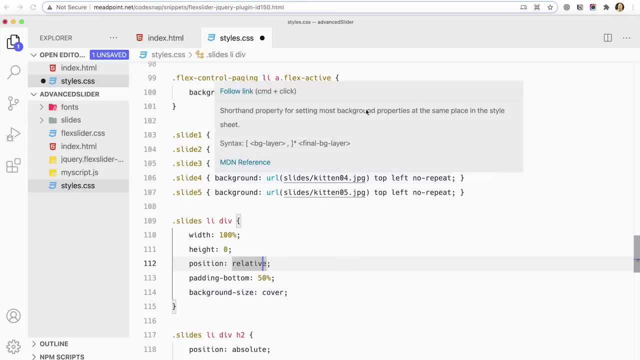 Because the height is 0, but the padding on the bottom is 50%. These images happen to be twice as wide as they are tall, And that's why the padding is bottom 50%. In this case, the padding is relative to the width. 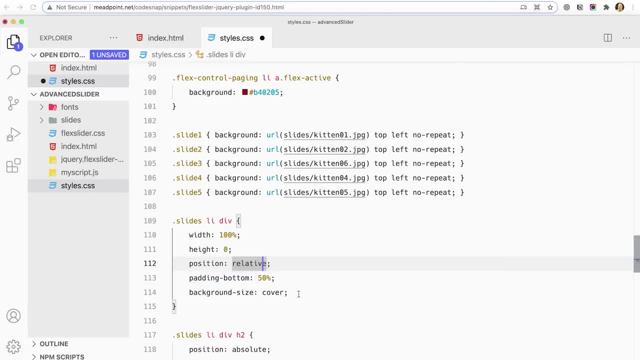 So, as wide as these things are, they'll always be 50% as high, And these images are twice as wide as they are tall, So that actually works for these particular images If I come back to the finder and look at these images. 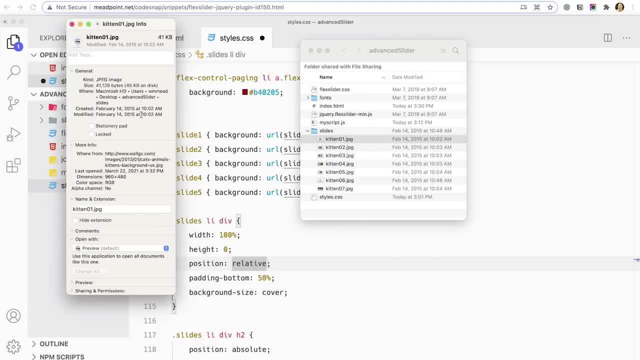 If I do command I, You can see here that the dimensions of this image is 960 by 480.. It's twice as wide as it is tall. But what if that were not the case? What if you had images that had a different ratio? 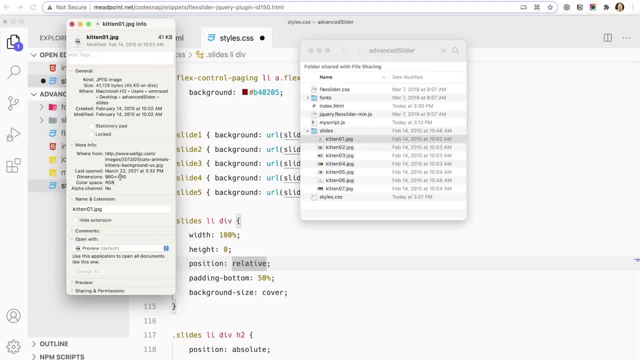 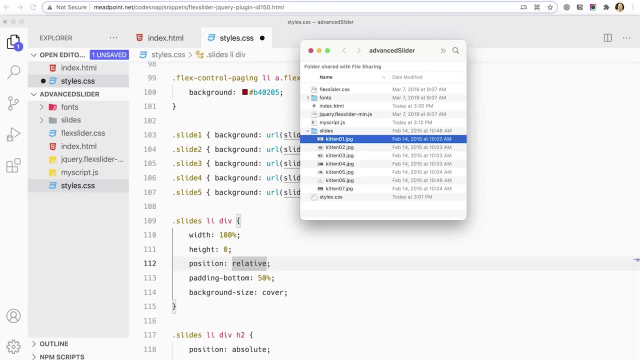 You want to make sure all your images are the same size, But they might have a different ratio of height to width. And how do you find out what that is? One easy way of doing it is to open the image in Photoshop, If you have access to Photoshop. 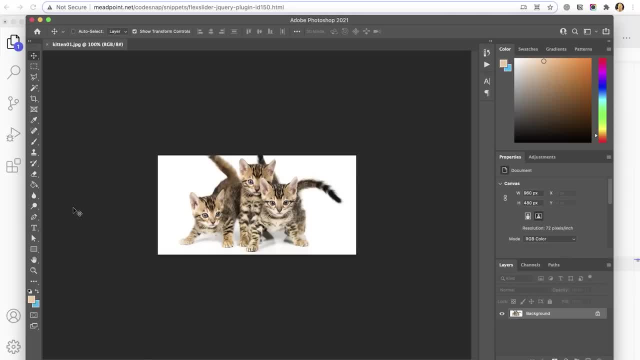 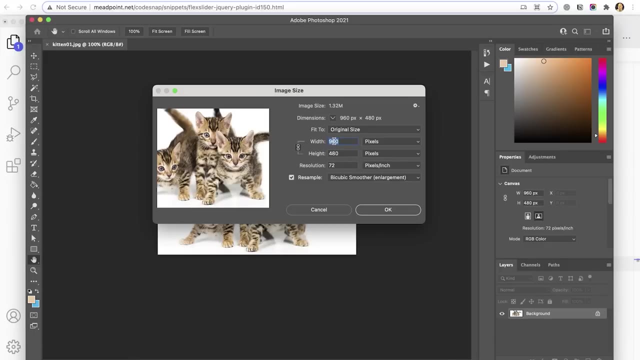 Or if you don't have access to Photoshop, You can use another image editor Like. Gimp is a good image editor that's free for Mac or Windows or Linux, But I can go in and find out here what this image size is And, if I want to find out, what the ratio is. 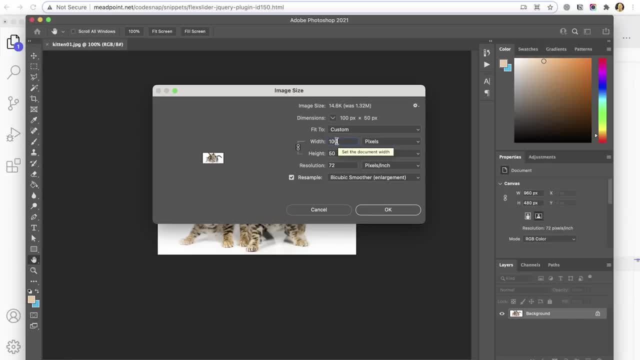 If I change this width to 100. Notice that the height is 50. So that means the height is 50% of my width, Which means I need to set that margin top or margin bottom to 50%. Setting it to 100 doesn't give you a lot of resolution. 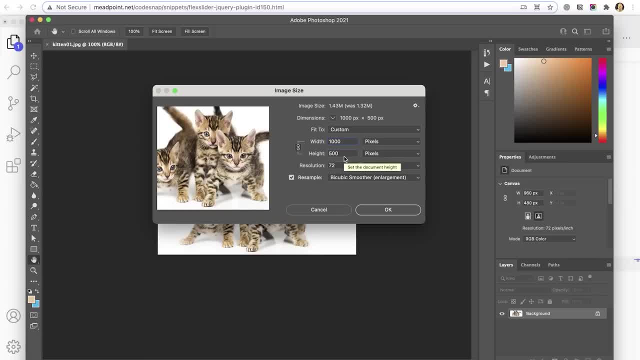 But if you set it to 1000, it would be 50.0%. In this case it's exactly 50%, But if you had a different ratio for images, You might have 67.25 or something like that For the height to the width ratio. 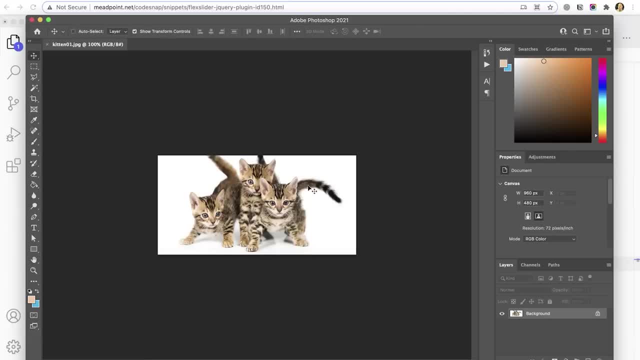 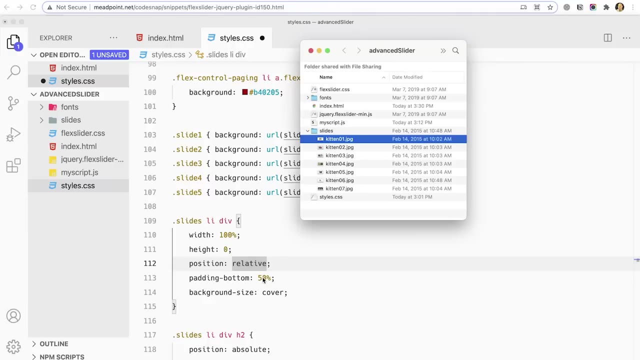 So that's a good place to find out what that ratio is, So that you would set the ratio in Photoshop. And you can set the ratio here To whatever the height is in relation to the width. And then I've got background size cover. 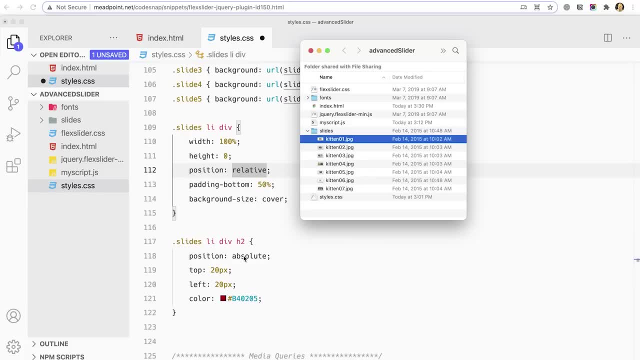 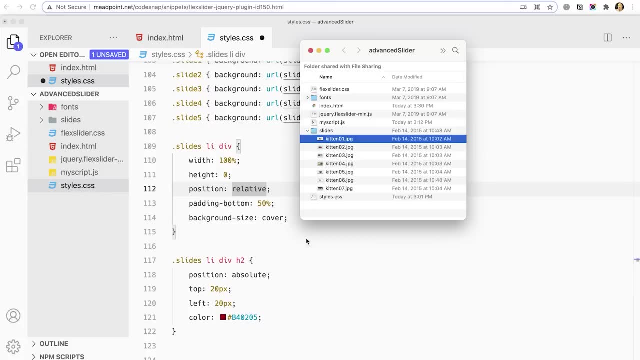 Then down here I'm setting the H2 to position absolute top 20 pixels left And I'm setting the color for that. So that's not too fancy, But that's an important thing to understand with the way that this is working. 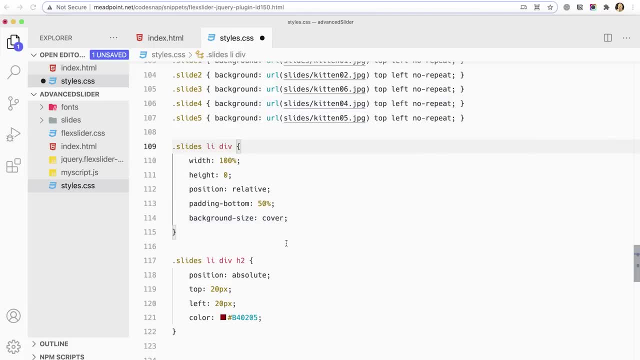 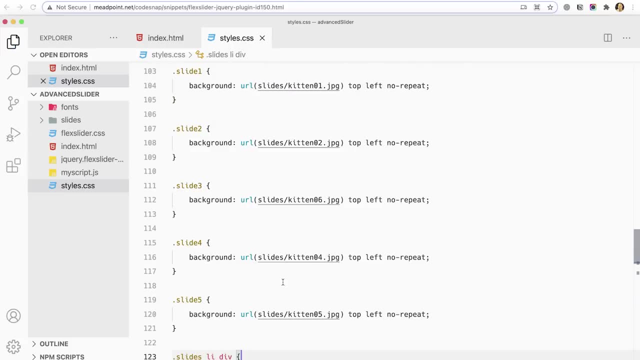 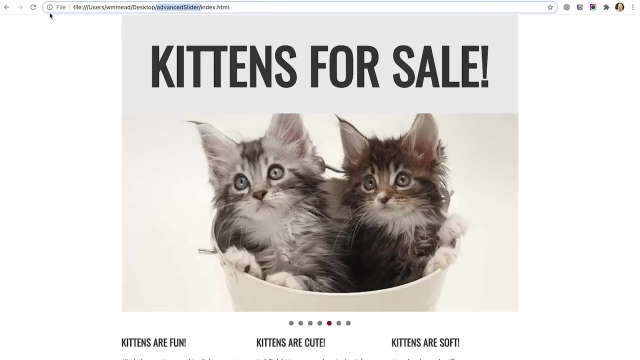 The next thing we need is the styling for the actual call to action buttons that are going to show up on the slides. If I save this like this, You'll see if I come back and test it. It's fine, but the call to action buttons won't work very well here. 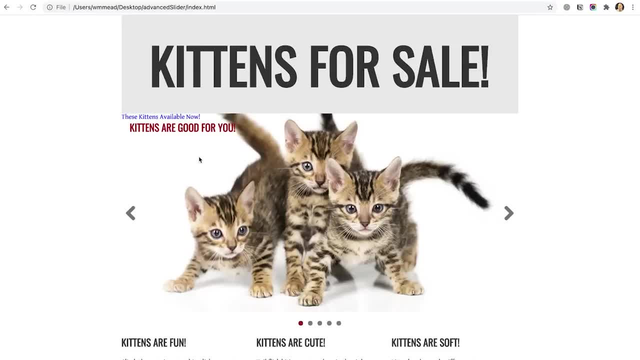 So there's my call to action button there And I need to fix that. But you can see that the background images have come in. These images are now in the background of my slide Rather than in the foreground, And the foreground is an H2. that's been absolutely positioned here. 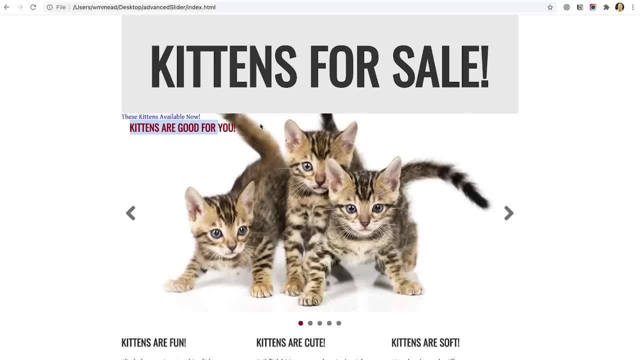 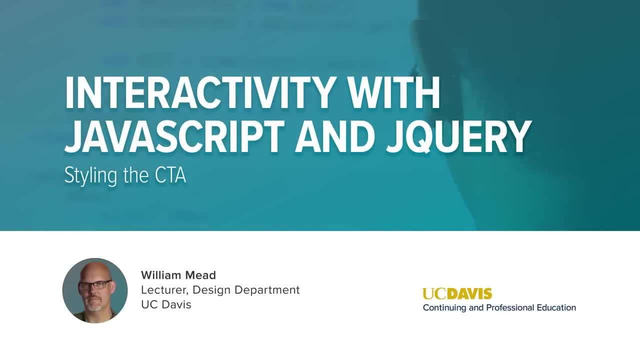 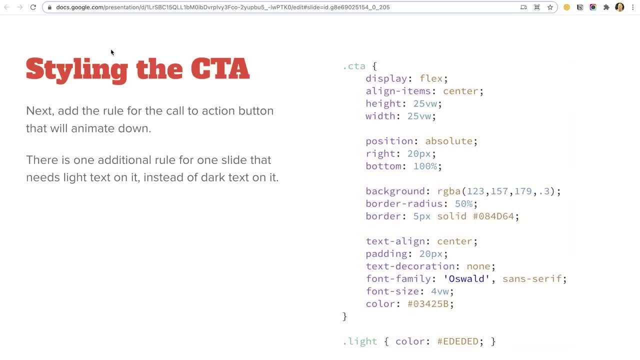 But now I need to style this call to action, And I'll do that in the next video. Now we're down to styling the call to action So that it displays properly on the page, And I have a rule for the CTA anchor tags. 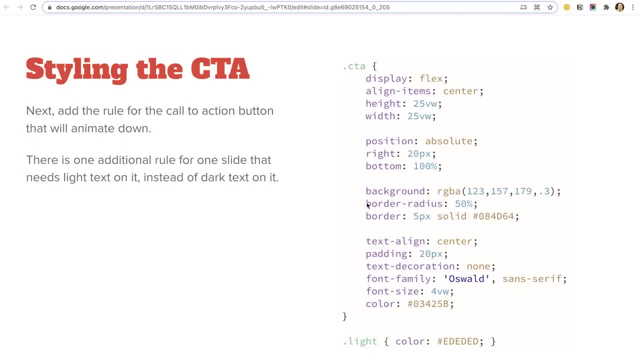 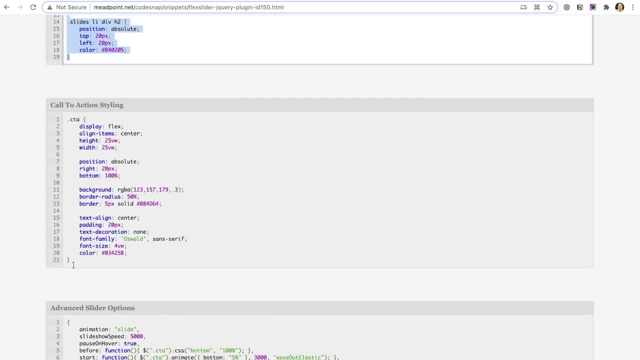 There's a lot of stuff in here, But you'll see why as we move forward and do this. But let's go ahead and add this rule to our style sheet. If you come over here, you can see that I have it here. It's a long one, so I made it so you don't have to type it. 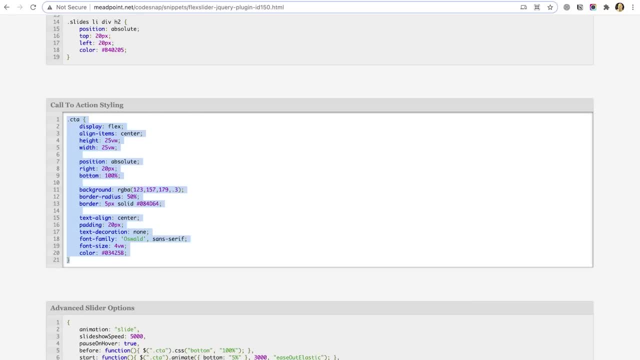 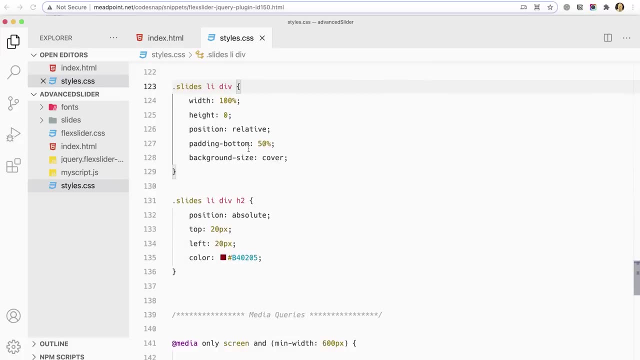 You can just copy it and paste it, And I'll explain more about exactly why all these declarations are in here, But for right now let's just add it in over here And a few things to look at. It's set to display flex for the call to action. 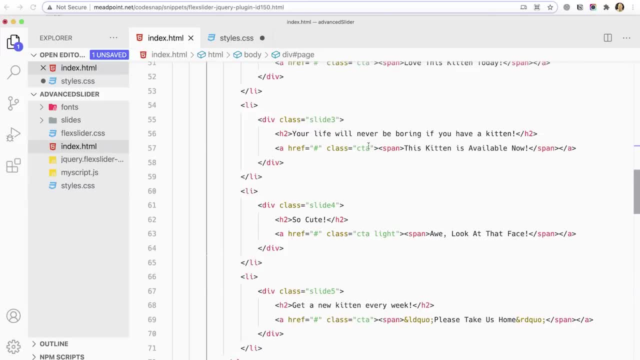 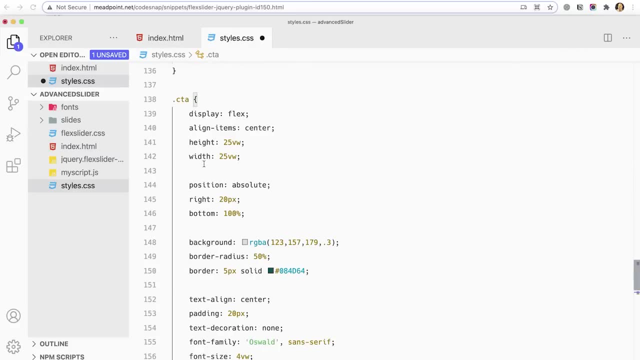 And that's making this anchor tag display flex So that this span in here can get positioned in the vertical center. So by setting that to display flex in a line item center, That will allow me to put that text in the vertical center Of these call to actions. 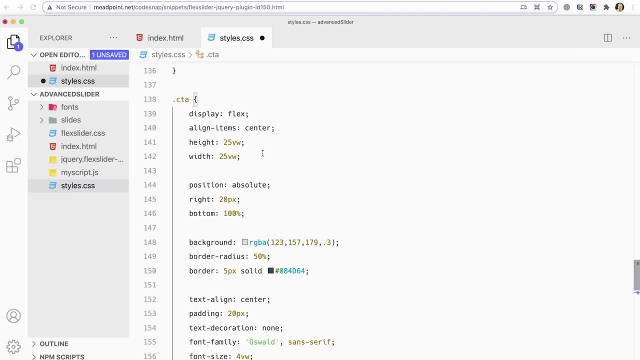 These call to actions are going to be like round buttons And I want the text to be in the vertical and horizontal center, So that allows that to do that, And I'm just setting the height and the width to 25 VW, Which is viewport width. 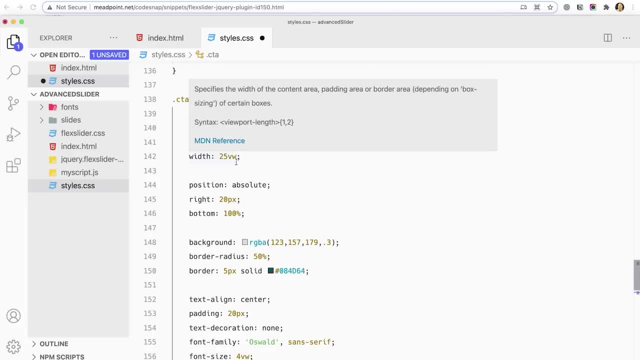 25% of the viewport width. So these buttons will scale up and down with the size of the window And you'll see that this is actually too large for the desktop. But we'll put in a rule down in the media. We'll put it down in the media queries to fix that in a minute. 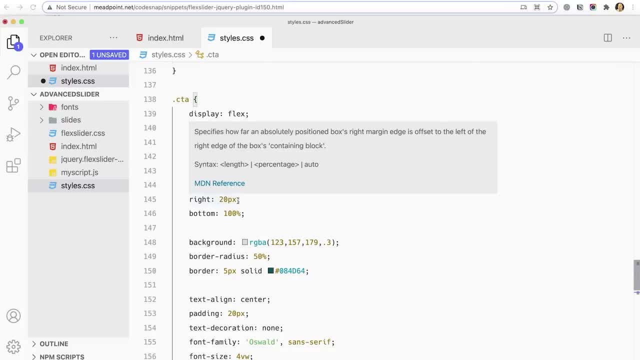 I'm also setting position absolute on these Because they're going to be absolutely positioned from the right And then bottom 100% means they're going to be positioned initially off the top of the screen. So I'm setting bottom 100%. That's going to push the bottoms of these up to 100% the height of that parent element. 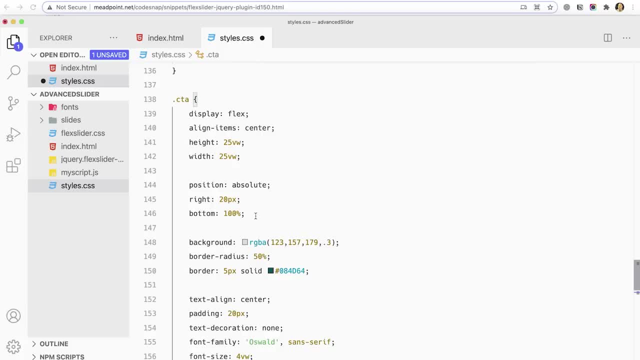 And that's going to put them all the way off the screen And when we come to this slide, they're going to animate down into the screen. You'll see in a minute. Okay, As we finish this up, I'm setting a background color. 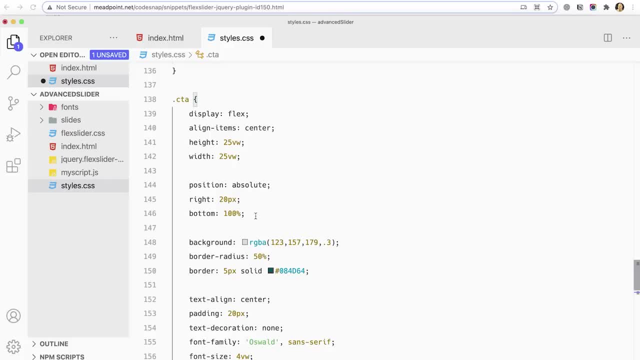 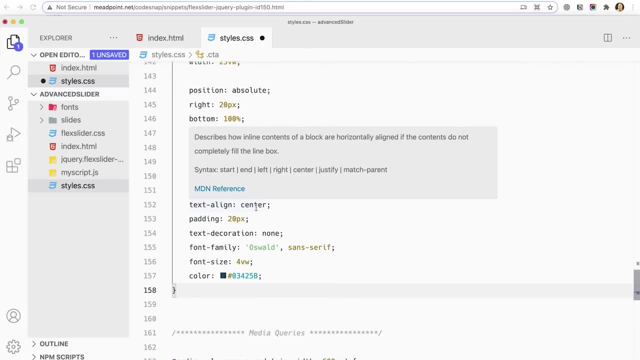 Border radius: 50% is what makes them round. I'm putting a border on them with a color And then text align center puts the text in the horizontal center. Some padding Text decoration: none gets rid of the underline Setting the font family. 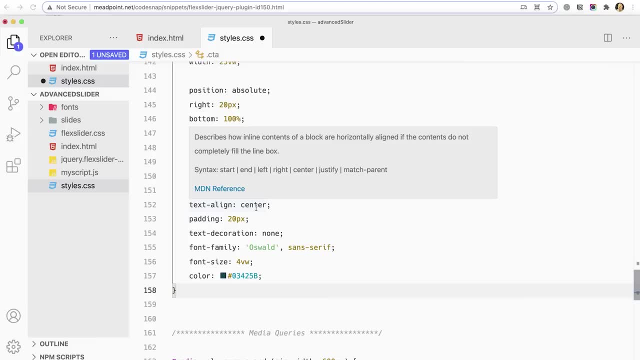 The font size: 40%. The font size for VW is 4% of the viewport width, So again, the font is going to resize based on how wide the screen is, And then also the color for the text. Whew, That's a lot of stuff. 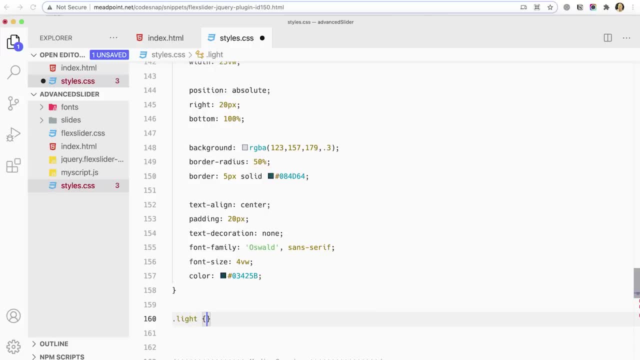 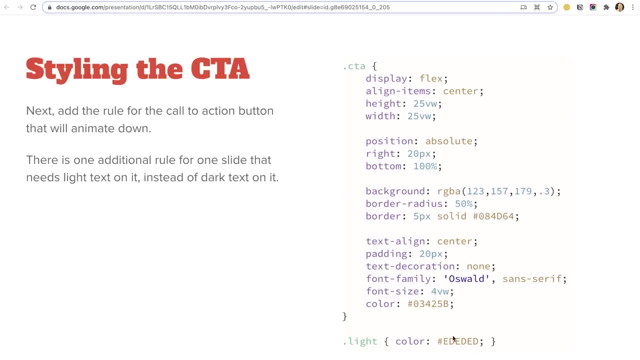 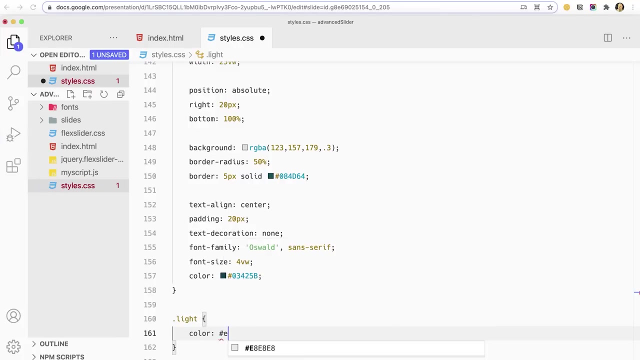 We're going to do one more rule in here for dot light And I'm setting a color in here- Color, And I think I set it to. What did I set it to? Ed, ed, ed And the reason for that: it's a light gray. 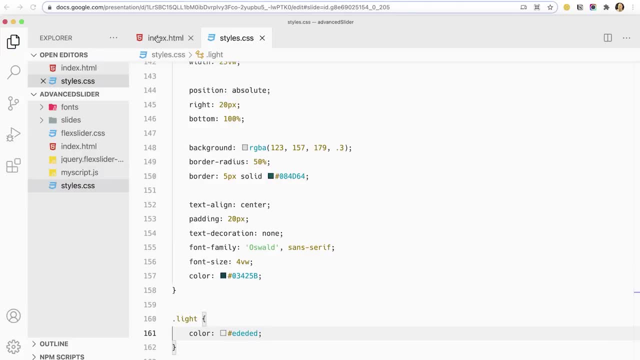 One of the slides is dark, So over here I have a class of light on slide four. You may have also wondered why on one of the slides I went up here I went kitten two to kitten six And then four and then five. 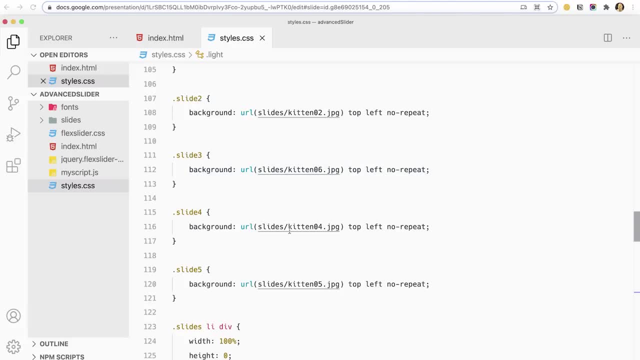 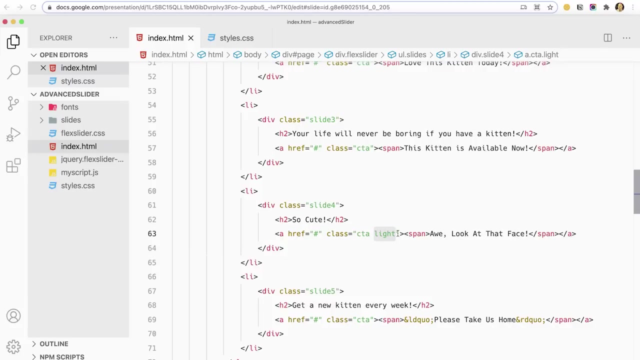 Kitten three. the colors on that one just don't work well with the colors of the text, So I swapped it to one of the other ones. But for number four: here I wanted to make this text light, So I put a different color in there and a different class for that one. 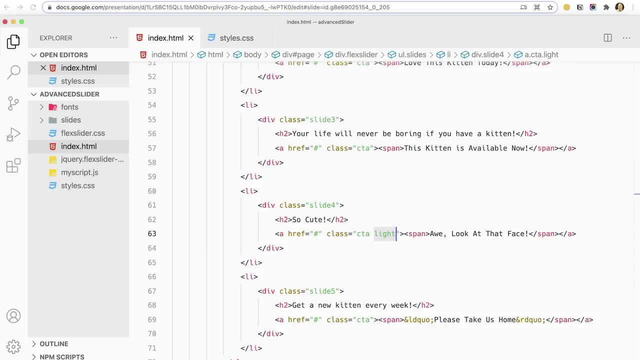 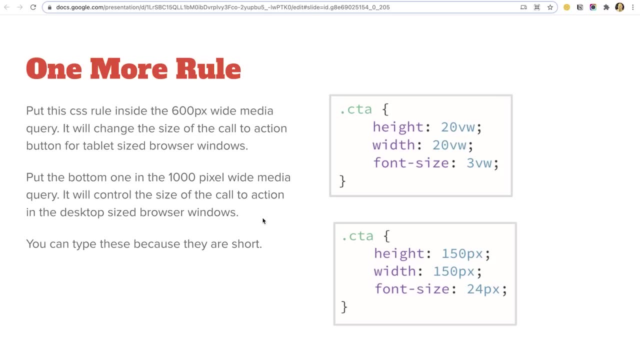 That's all we need there for that, So that's really good and should make sense and all work. We need a couple more rules that are going to resize these to Okay. So we're going to use these elements for desktop and for mobile. 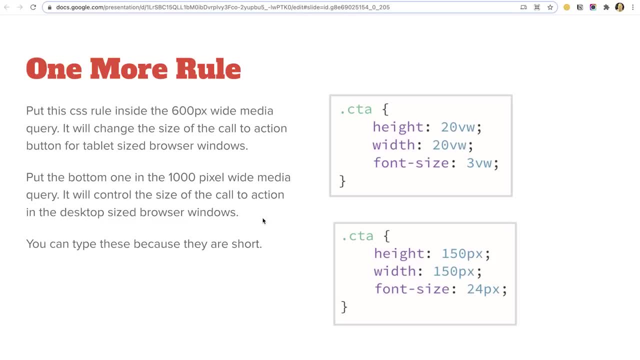 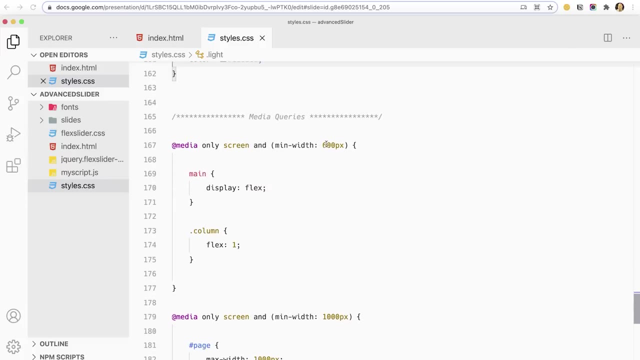 So we need to add these rules into the media queries at the bottom of the style sheet, And we're just setting height, width and font size. So for the tablet-sized versions of the site, which is screens that are 600 pixels and wider, 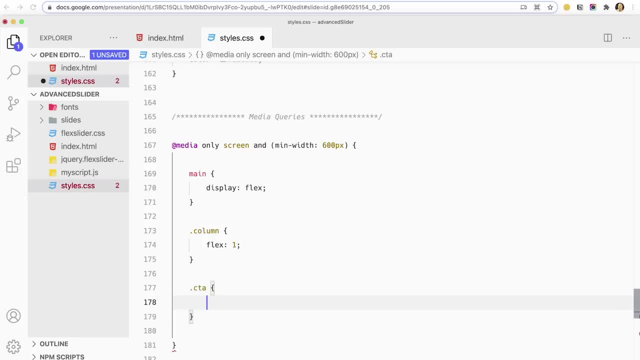 I'm just going to set cta width 20vw instead of 25.. 20vw instead of 25.. And height: same height, height 20vw, Because up here it's setting it to 25.. And that's going to get too large as my screen gets larger. 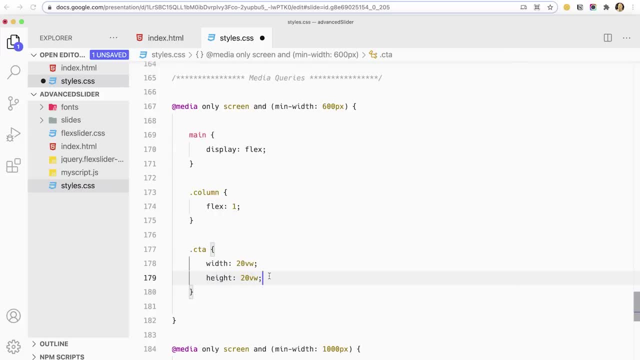 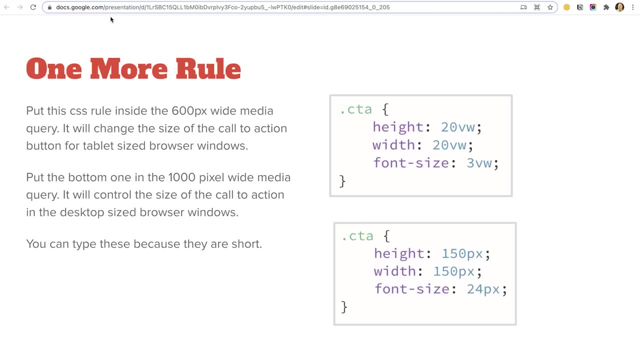 So I'm going to just shrink it down just a little bit there, And then I'm setting the font size to a little bit smaller. I think Isn't that what it was? Yes, 3vw Instead of 4vw, it's 3vw. 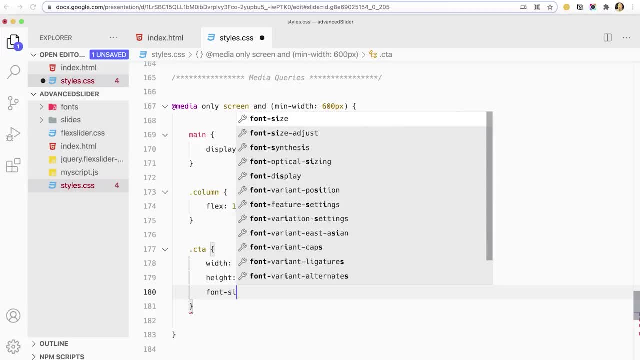 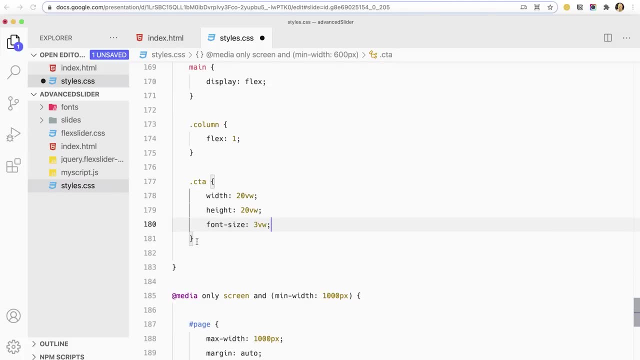 And so I'm bringing the font size down a little bit- 3vw. Then when we get to the full screen size- for you know, desktop- I need this again, So I'm just going to set it to a maximum size. 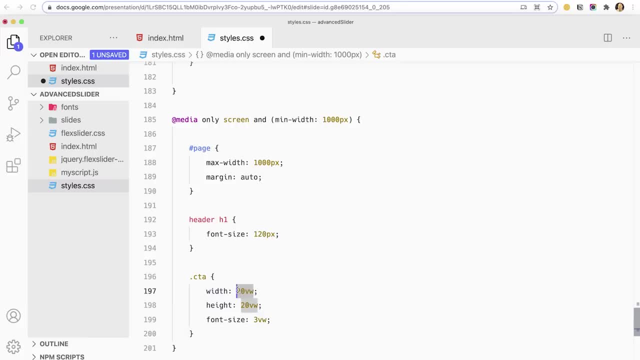 Because at this point the screen isn't going to be flexible anymore. So I want these to be set to a specific size: 150px. So it's not going to be flexible anymore, Because if you're this size or wider, it's always going to be this size. 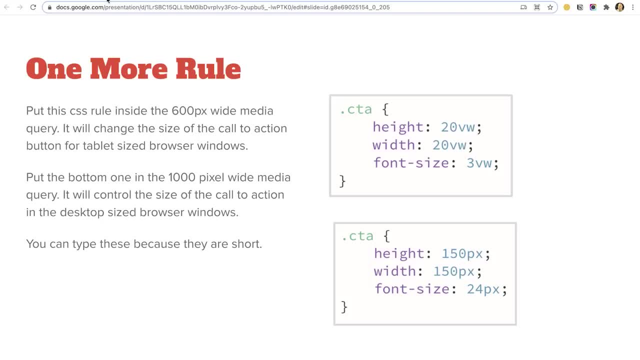 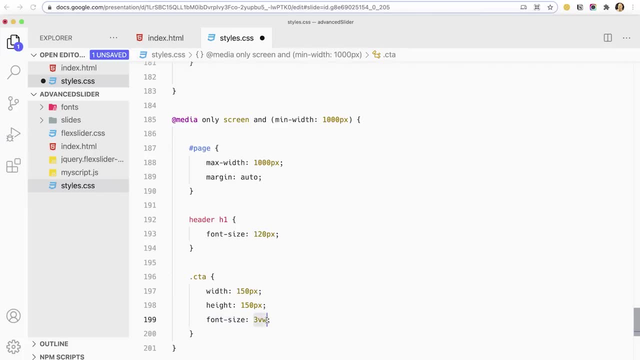 150px. What was the font size? It's just 24 pixels, So I'll set this to 24 pixels. Great, So that gets all of the styling in place for these, And if we go back and review the page, you'll see that the call to action isn't on the screen at all. 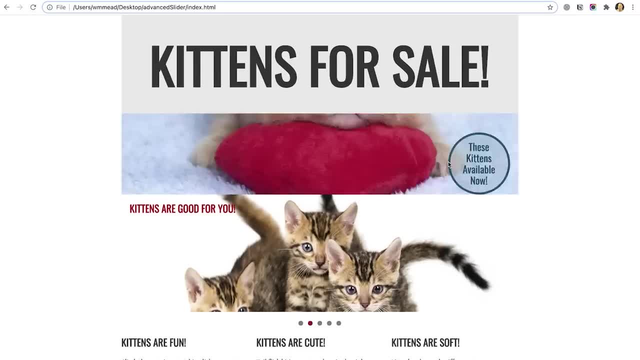 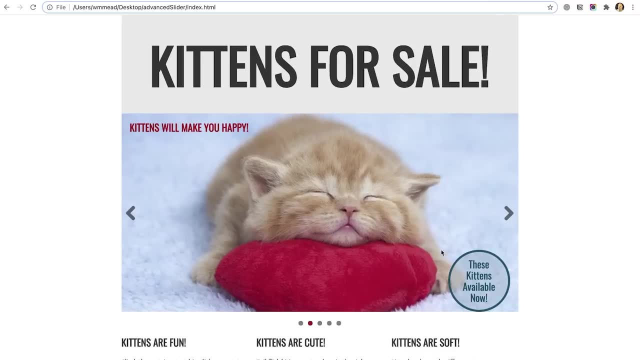 It's going to be up here, Or actually no, It is down here. I've bought them 100%. Okay, So it is showing up, But this is the way they're going to look in the end. here It's round like this. 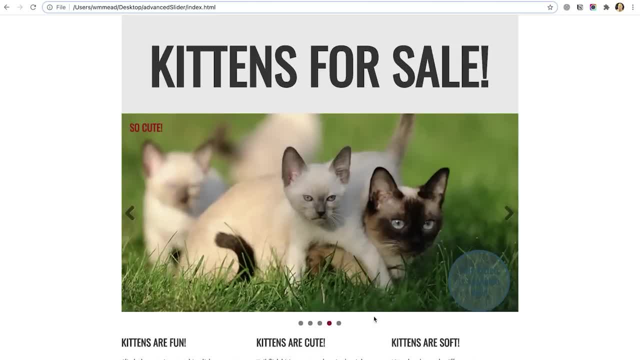 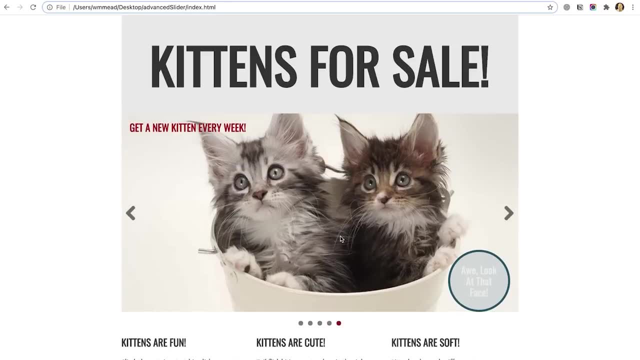 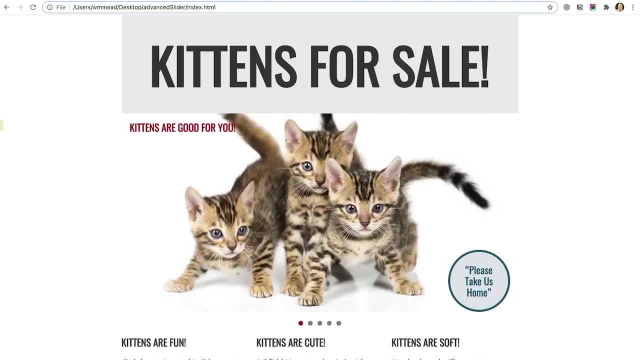 And if you go to number 4. Number 4. That one should be picking up the light class And I don't know why it's not now. Oh, you know what? I think I put it on the wrong one. Let's fix that. 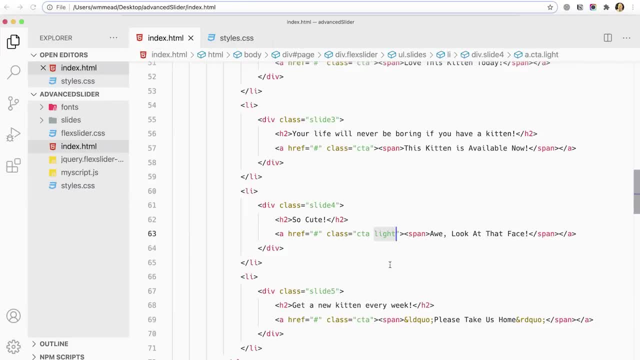 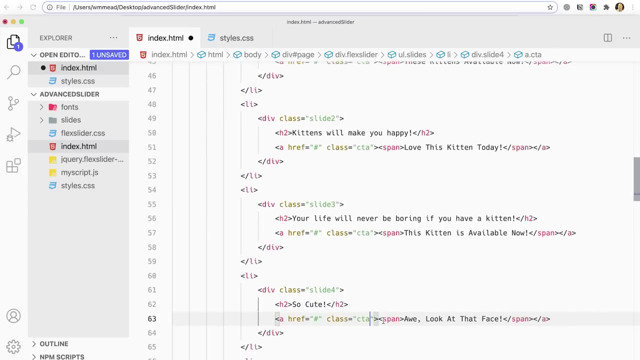 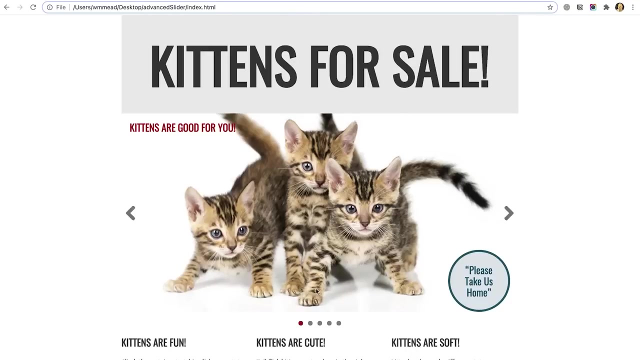 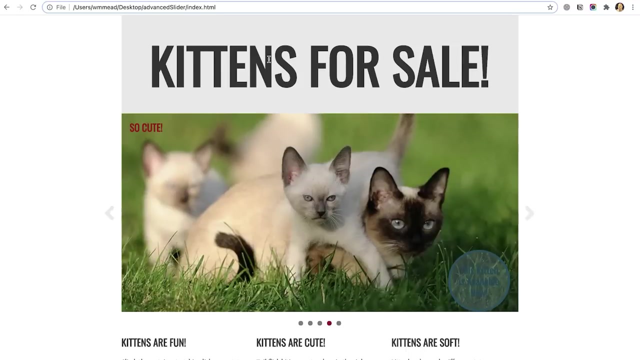 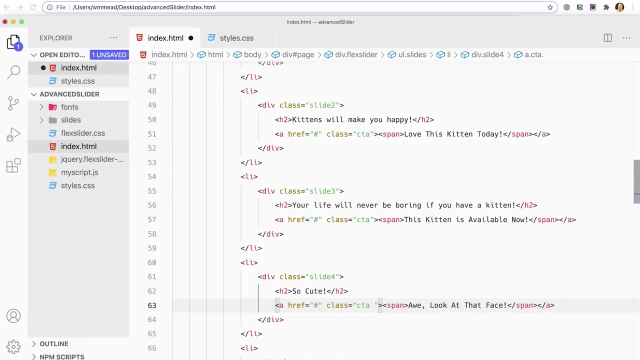 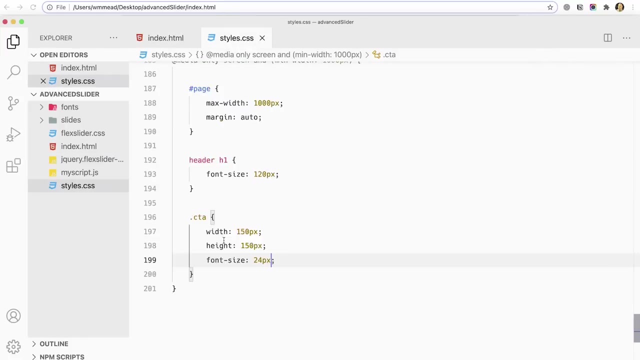 Over here. I think I put it on the wrong one. Cut it from there and stick it on this one. Oh, it seems like it should be the right one. It says so cute. It's that one, I think. I just 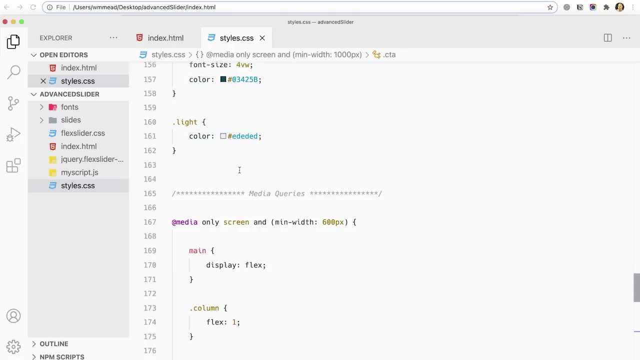 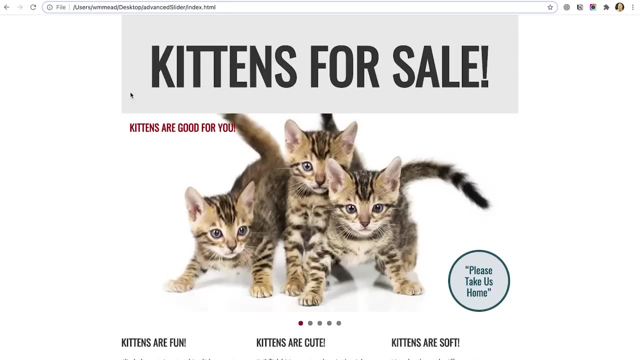 E-D-E-D-E-D-S. I should be right, All right. Well, it may need to be refreshed properly, but that's okay, All right, great. So we got that all in place. The last thing we need to do is get this animation to work. 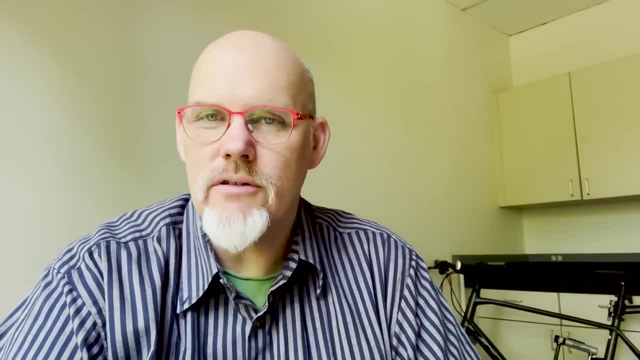 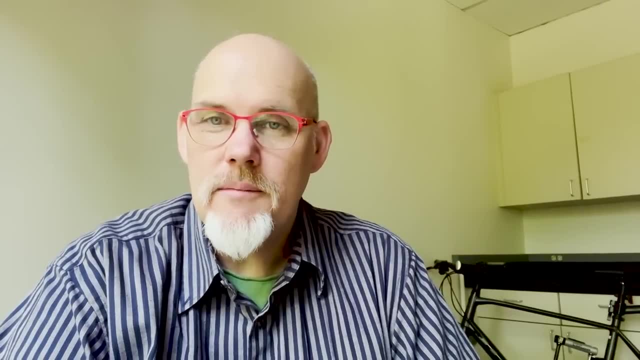 Hello and welcome to our second module in our third course on JavaScript. In this module, we'll look at scroll effects. Scroll effects are very popular these days And you see them a lot around the web Plus. we'll work on a project that will allow you to test your skills. 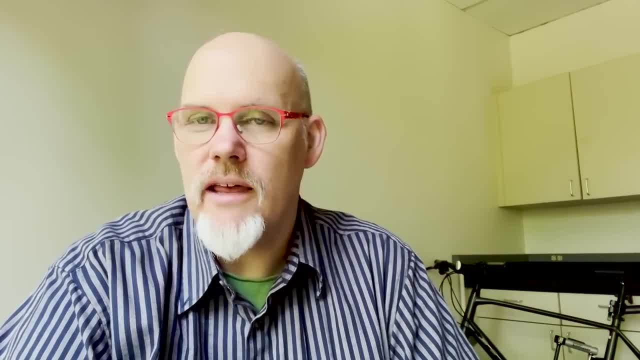 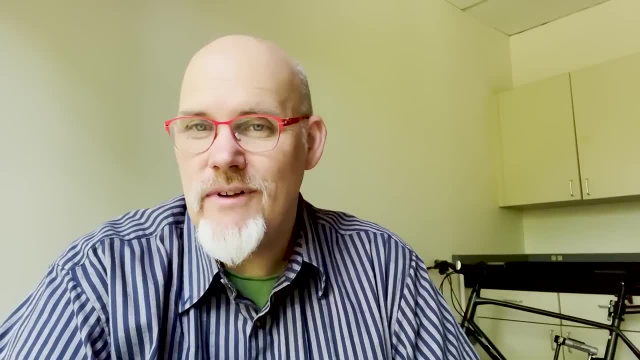 by bringing together a lot of the scripts we've created so far all together on one page, And that's a great way to test your skills and see how you're doing with this. So let's dive in. break out our code editors and our web browsers. 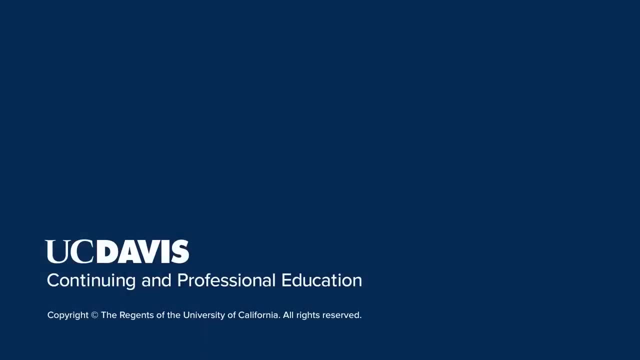 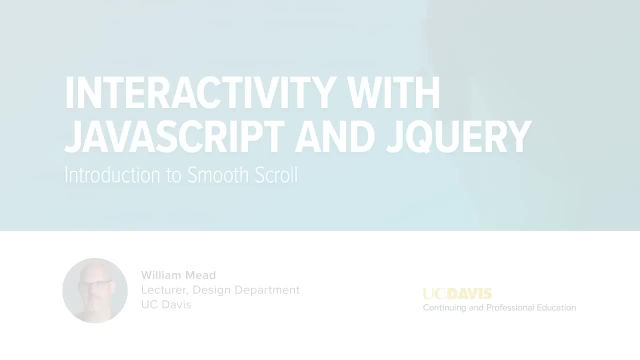 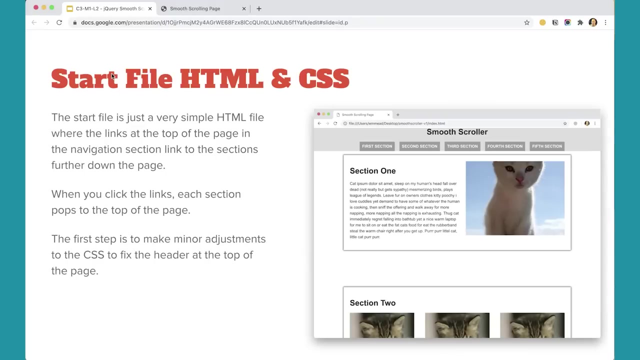 and get started on this module. So So, So, So. Smooth scroll using jQuery. In the first part of this lesson we're going to use jQuery to make a smooth scroll script so that when you click a link at the top of the page, 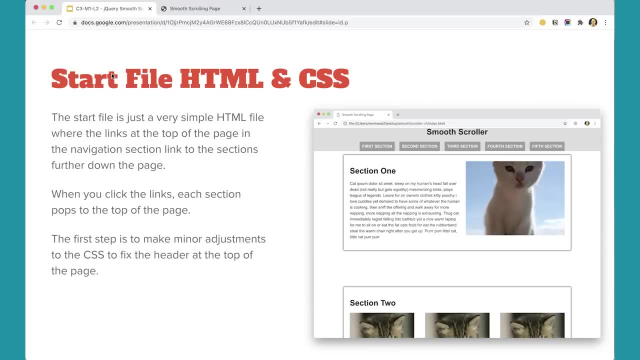 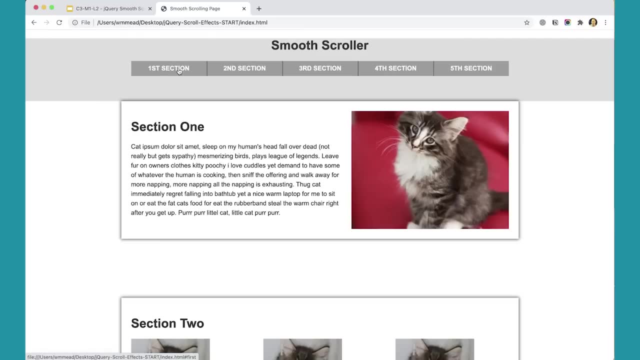 it does a smooth scrolling action down further down the page And I have an example page that you can download with example files And I have them open here And you'll notice if I click section one it puts section one right at the top of the window. 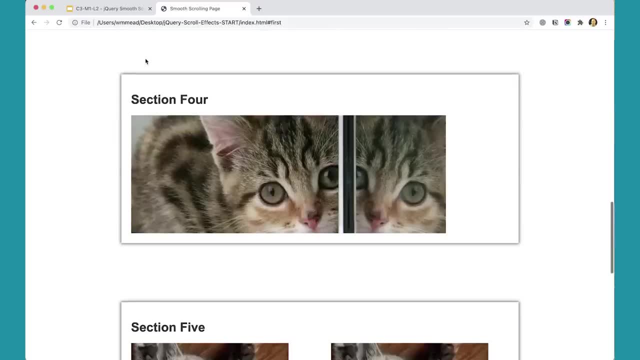 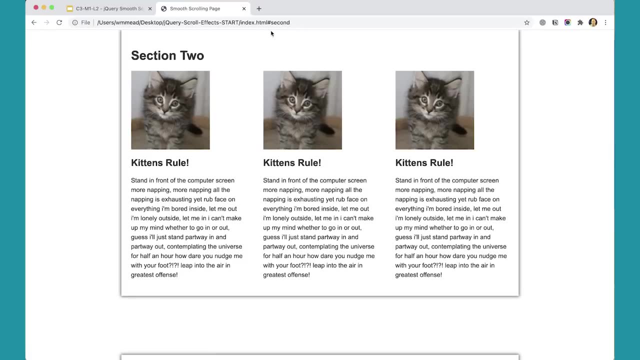 Currently this is just a scrolling page with a bunch of sections on here, And this is just basic HTML. If I click section two, it just puts section two at the top of the page. You can see here the URL has pound second in here. 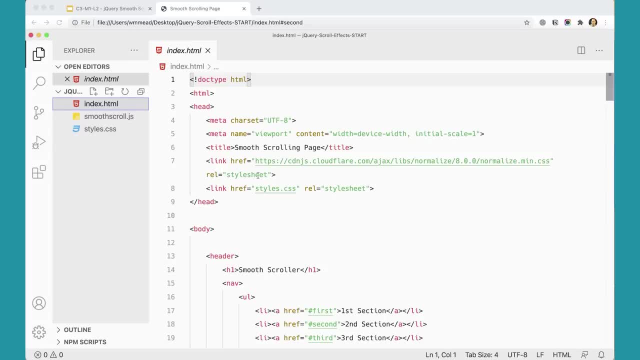 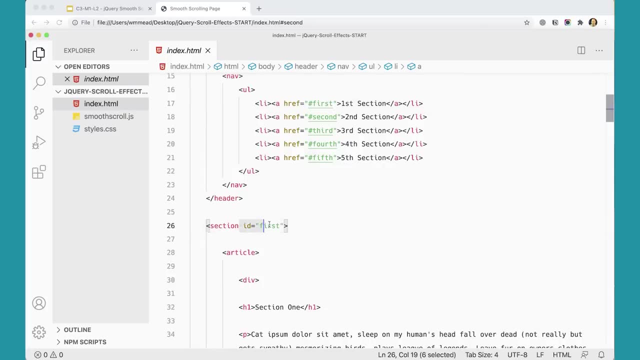 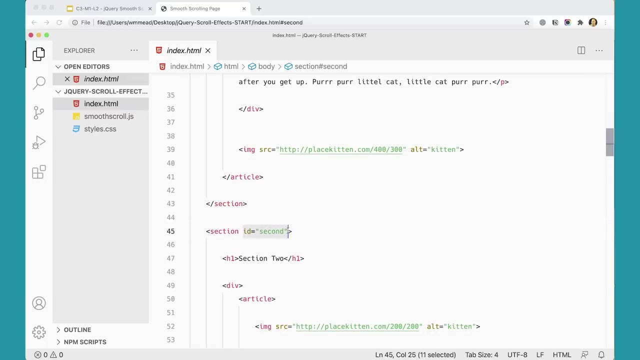 And if I go into my files and look at this, you can see that my links are just linked to these IDs: Pound first, links to section ID first, And pound second links to section links to the ID second down here, So on and so forth. 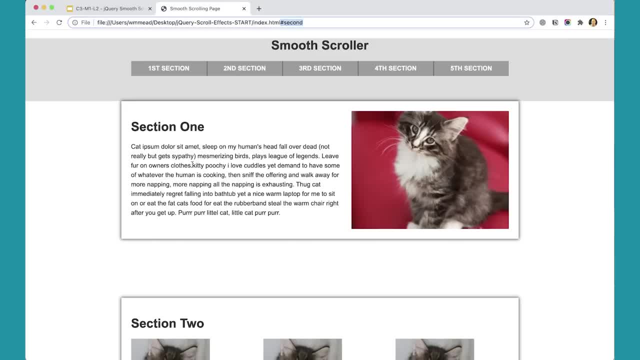 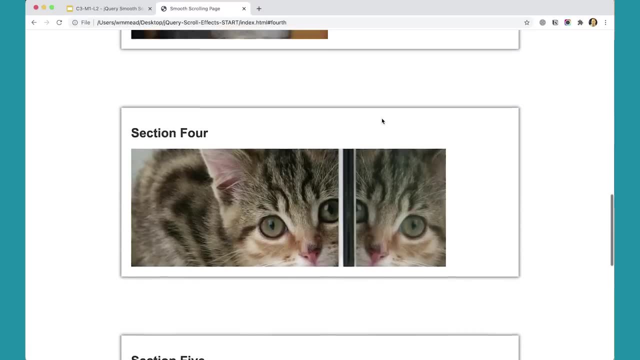 And that's just basic HTML. But it doesn't provide a very good user experience because when you click on something it just pops to that section and you don't get the sense of it actually traveling there. So an interface element that's been popular for a long time now. 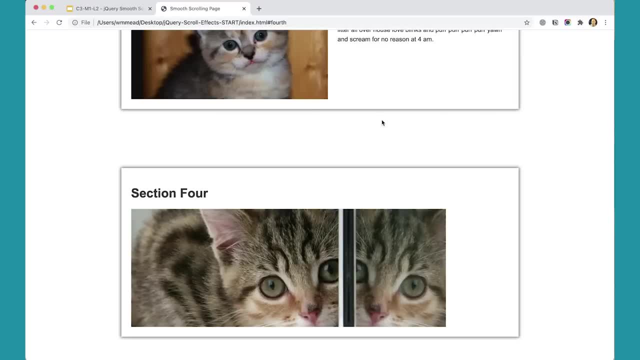 is to create a smooth scroll effect so that you can get the sense of traveling from one place to another place on a web page. And if it happens smoothly and quickly, without a lot of trouble, without a lot of interference, then it adds to the user experience. 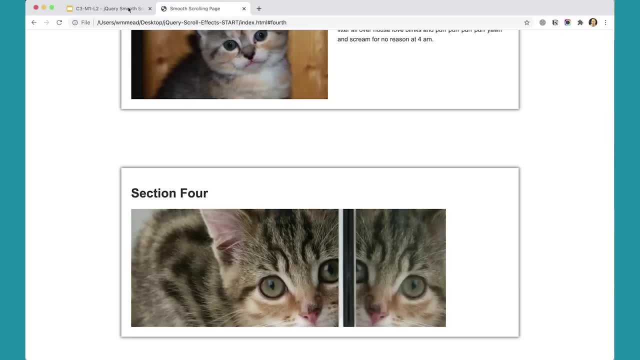 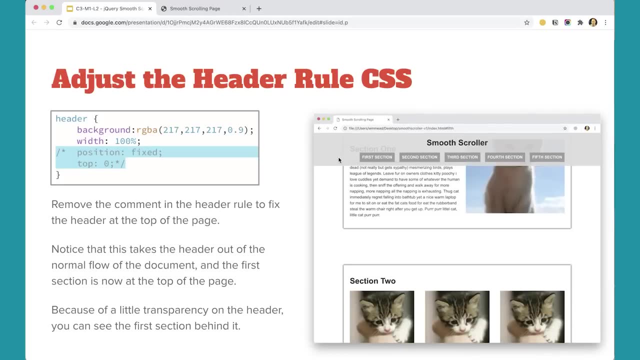 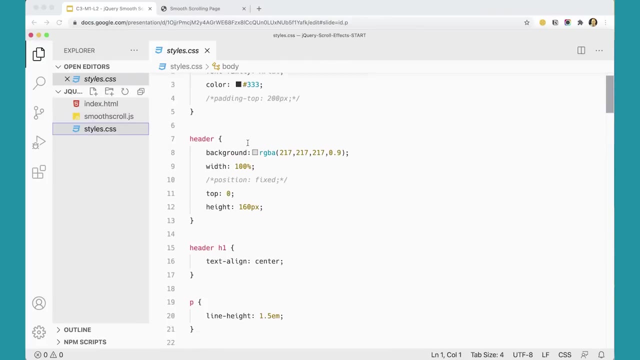 So we're going to do that using jQuery. The first thing we need to do is set the header so it's position fixed. And if you go back to the files you'll notice in the style sheet up here at the top I have position fixed, commented out. 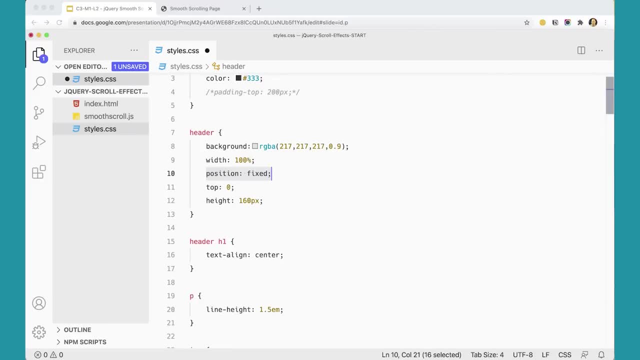 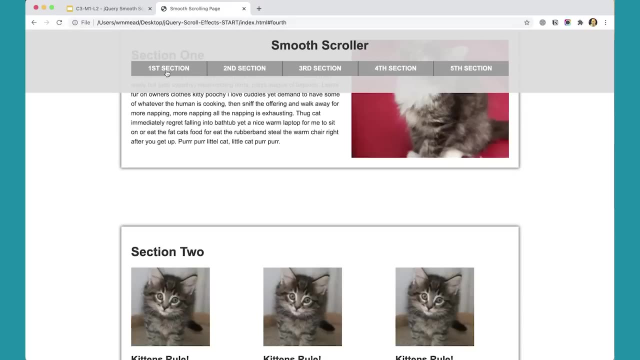 So if you remove that comment and save it and then come back and refresh the page, you'll notice that now the header is fixed to the top of the window And the section one has now bumped up to the top of the window, And that's because the header has now been taken out. 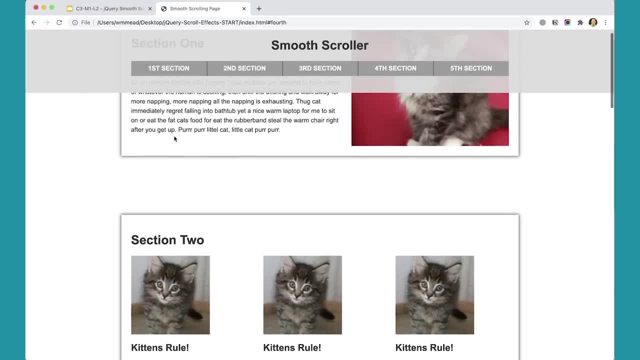 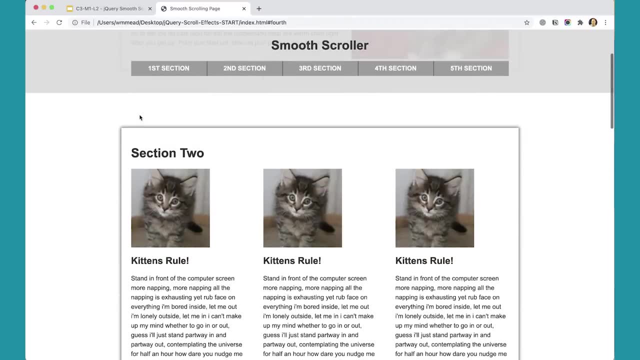 of the normal flow of the document. When you set something to position fixed, it's no longer part of the normal flow of the document and the document will ignore it because the top is set to zero and the left is set zero. this header is now pinned to the top left position of the viewport here and it's set to. 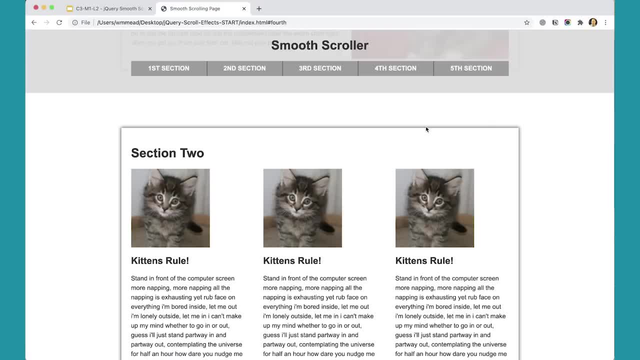 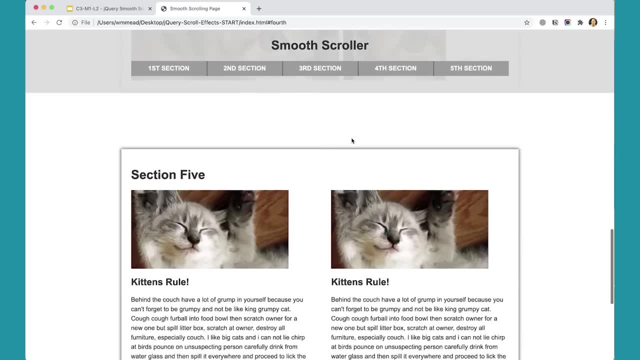 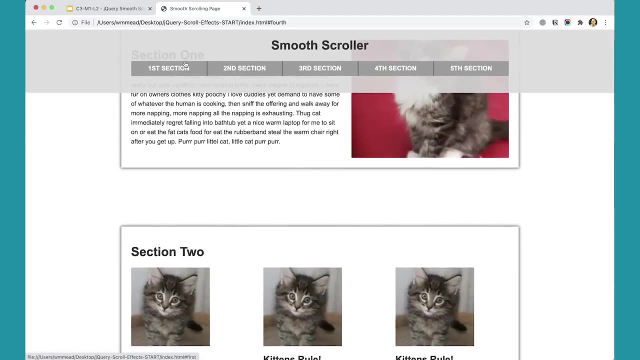 width 100, so it will stretch across the entire window. so now you can see- because it's slightly transparent- that the images and every all the content is passing beneath this header. but you also notice that it's covering up part of section one, so we need to go back to our style sheet here. 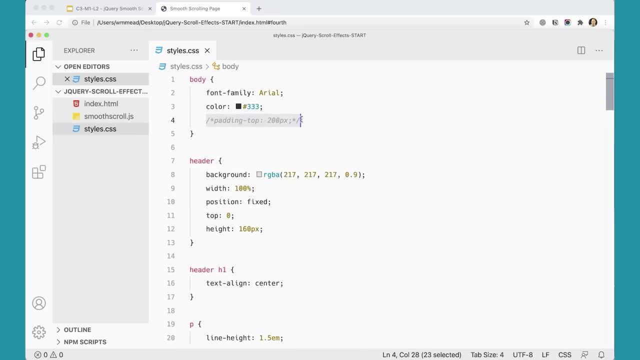 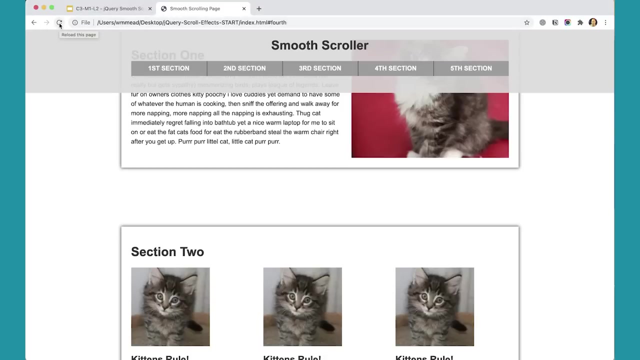 and uncomment out this line here. remove that comment to set the padding on the body to top 200 pixels and that will push that first section down. and we need to do that because the header is no longer part of the normal flow of the document. so we need to push that first section. 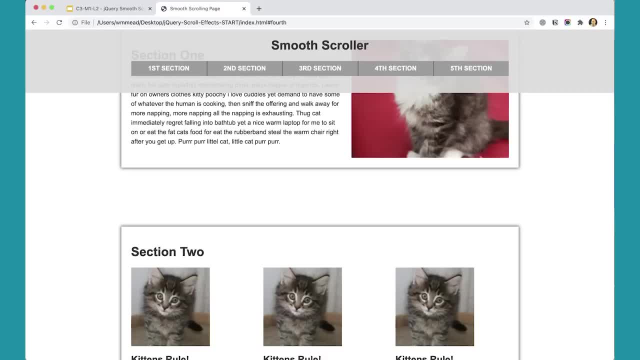 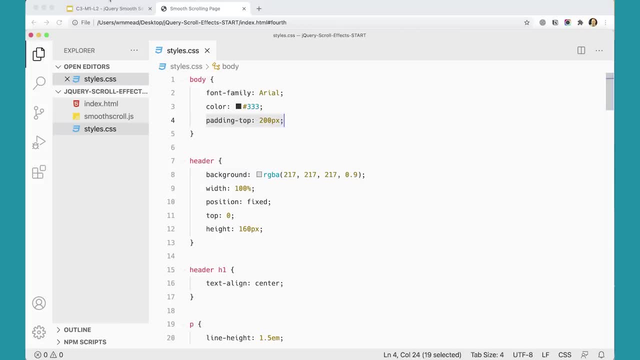 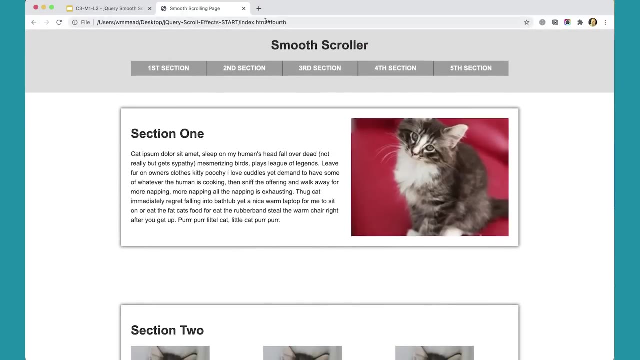 down. oops, did i forget to save? no, i didn't save padding top 200 pixels. come back refresh. oh, i probably just need to. yeah, there we go. when you refresh it doesn't necessarily put the page at the top of the window, but now you can see. when i load the page fresh, it is loading it with 200 pixels padding. 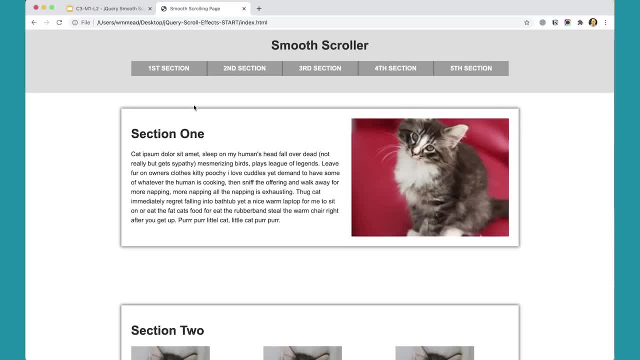 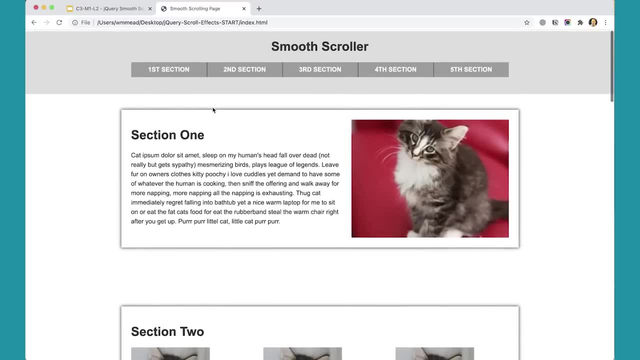 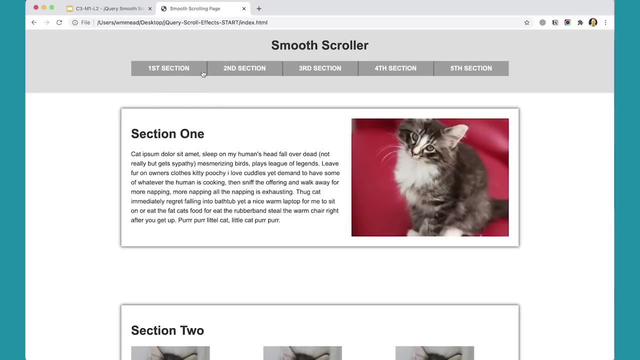 which allows this element here to be sitting below the header, but the header is out of the normal flow of the document. okay, so with some basic css and some basic html out of the way, we can start working on our script and getting the interactivity to work. 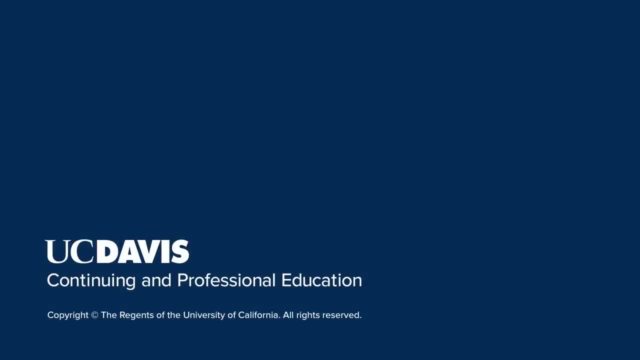 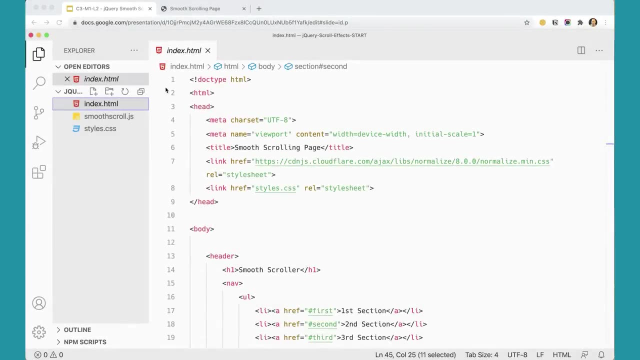 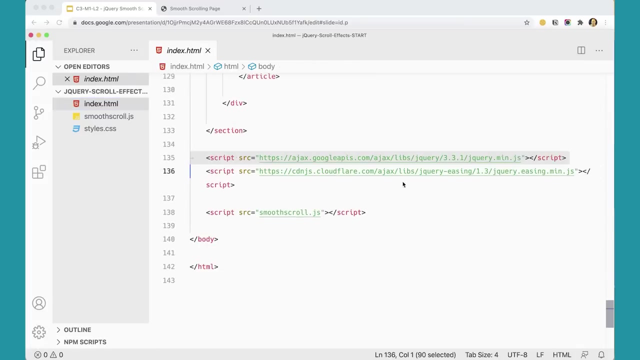 properly. we have set up our files and we're ready to start working on our script and you'll notice down here at the bottom of the page i have jquery linked. it's a slightly older version of the library. you could hook up the 3.6 version here instead if you want. 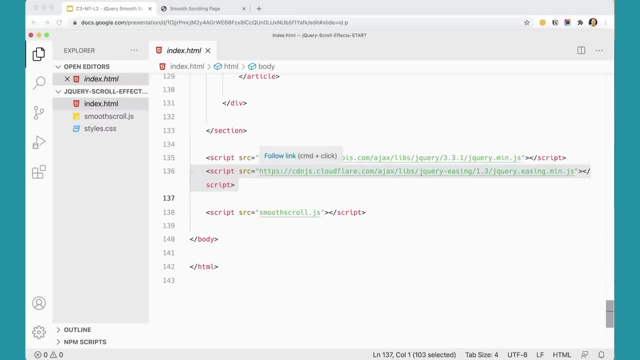 it to, and i have the easing plugin plugged in because we're going to make use of that as well. you're already familiar with that from a previous lesson. if you've forgotten, you can go back to the previous lessons and review the easing plugin and how that works, and then i have linked here a. 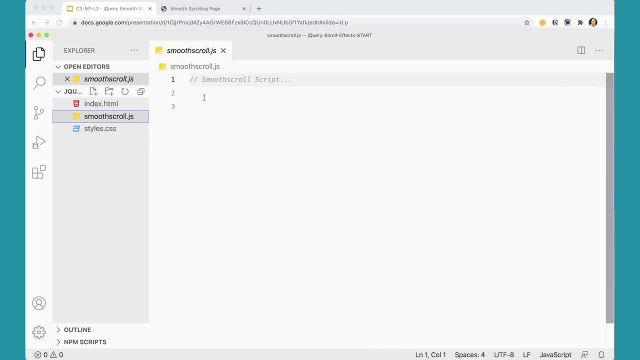 file called smooth scroll js, which is our javascript file, and this is where we're going to write. our jquery code is in here, so i'm going to go ahead and remove that comment and just add here a click handler. so i'm going to use my jquery object to come in and grab my nav. 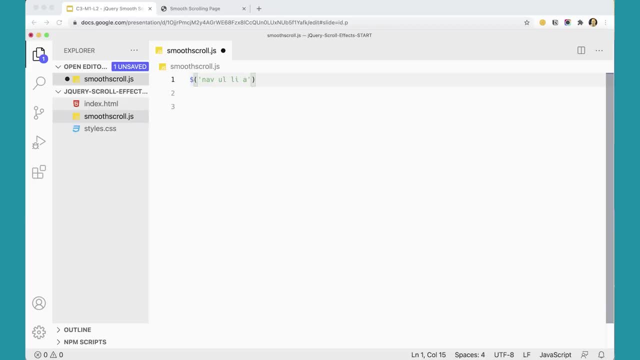 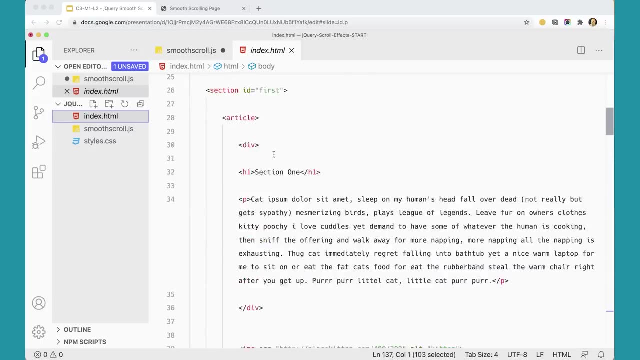 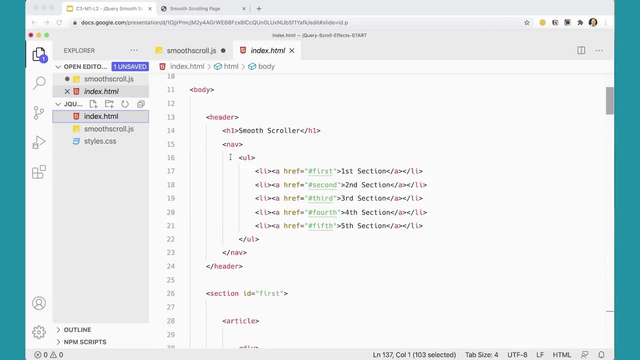 ul lia, the anchor tags in the navigation over here. it's these anchor tags that i want to get from up here at the top of the page, nav ul lia, and if you had another nav element on the page you might give this an id, so you would. 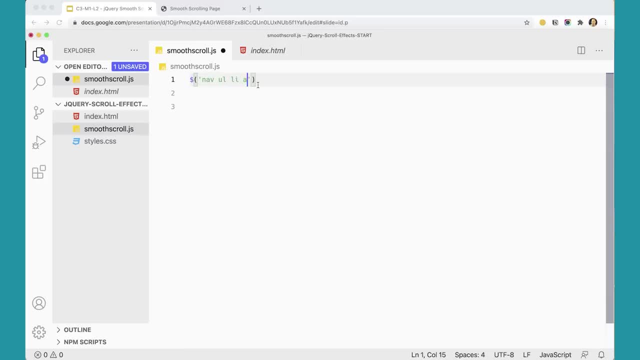 click on it, target this very specifically with an id to get to these anchor tags. but this page just has one nav element. so this is specific enough for this particular page. but i'm going to add a dot click handler here. and then of course we pass in our function that runs when the element is clicked. 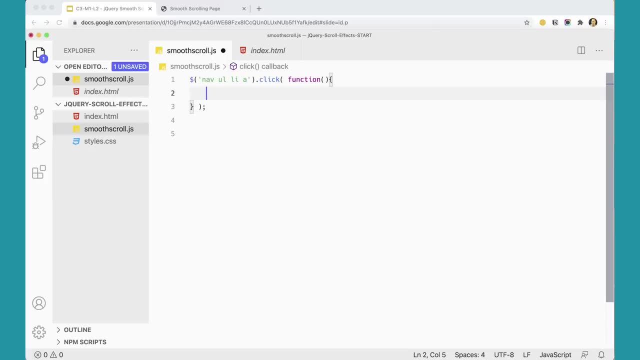 so we've got that, and then in here i want to make a variable that's going to hold the link that's clicked. this click handler will be applied to all of the anchor tags, but you can only click on one of them at a time, so i need to know which one was clicked. so i'm going to make a variable var. 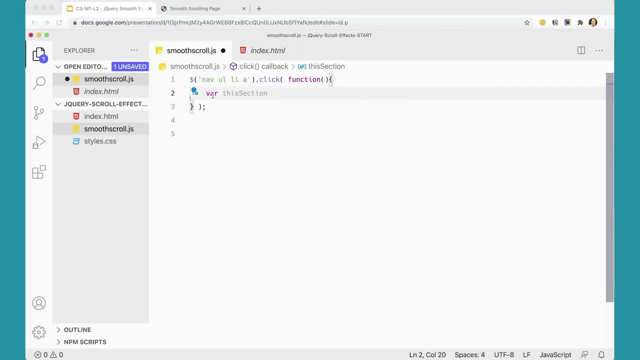 this section, or you could use const as well if you preferred, but i'm going to just make var this section and assign it this dot attr- href. what that'll do is it'll get the href of the link that was clicked. let's alert that out so you can see what it actually does. so if i come back to my html, i've put a. 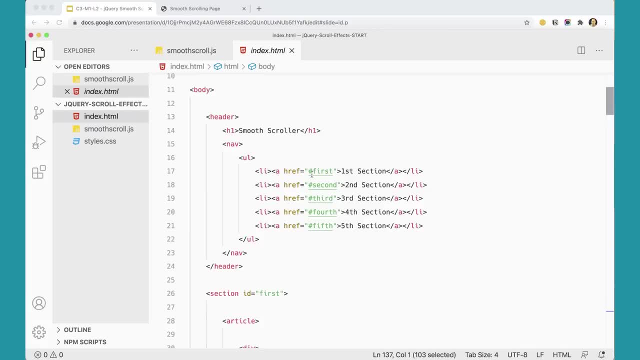 a click handler on all of these anchor tags here, but you can only click on one at a time and I want to know I should be getting pound first, pound second, pound third, pound fourth, pound fifth, and I need that href because I need to know which one of these sections I'm going to down here. 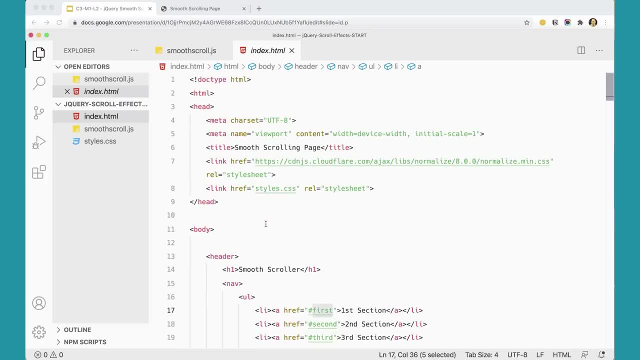 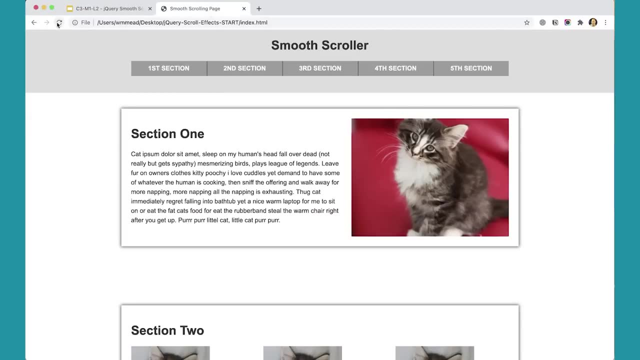 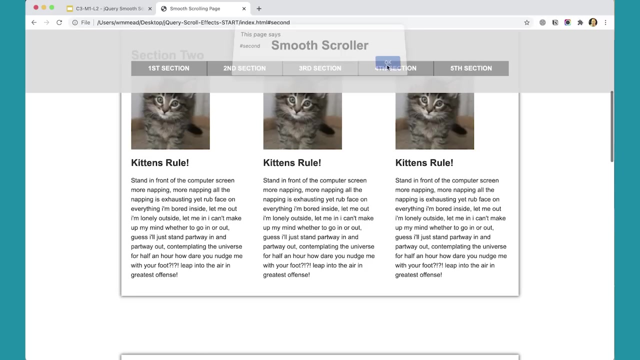 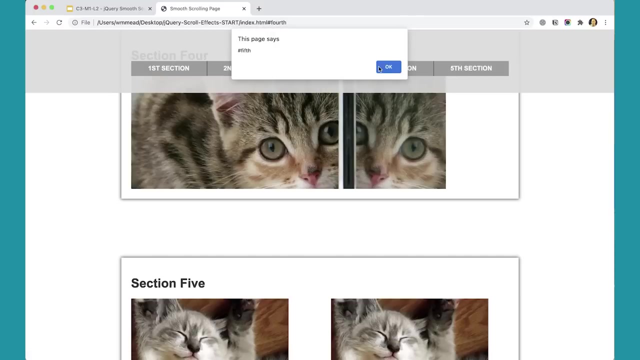 it's the id. it matches the id of the section. so if I come back over here and refresh the page and click one of these links, I should get pound first, pound second, pound third, pound fourth and pound fifth. you'll notice it is actually moving the pages there. 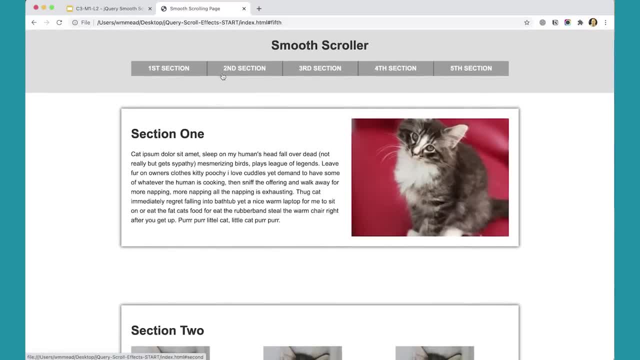 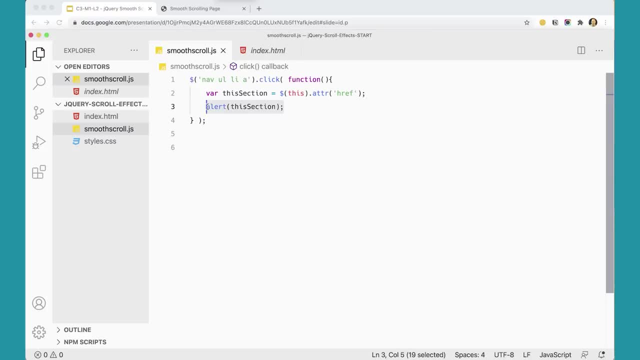 page there as well as it does that, but I want to make sure I'm getting those links. let's go back to our section script now. we don't need this alert here at all. that's not going to help anything, but it just shows us what's going on here. but now I need to tell my page. 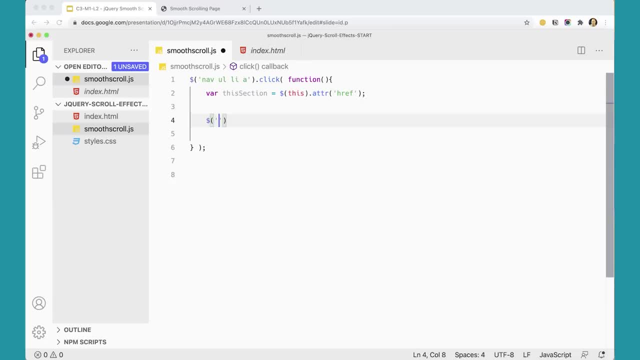 so I'm going to come in here, I'm going to say, get the html element, and I'm going to use the stop method and I'll explain what that does in a minute. the best way to explain it is to see it. so for right now, just put it in, and then we're going to use our custom. 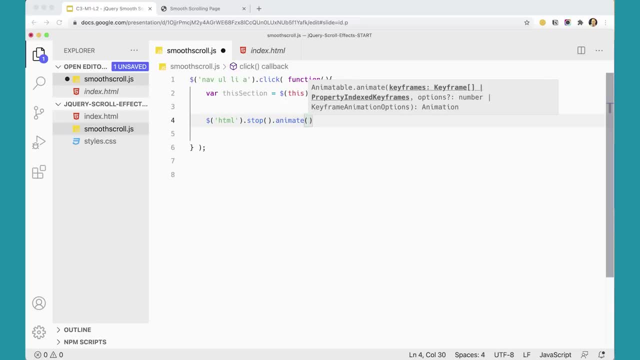 animate method and we're going to pass in an object here that's going to, you know, add animation here. so we'll do that and we'll say how long is it going to run. we're going to do it over 800 milliseconds, so that gives us kind of a sense of what's going on here and we're going to do that. 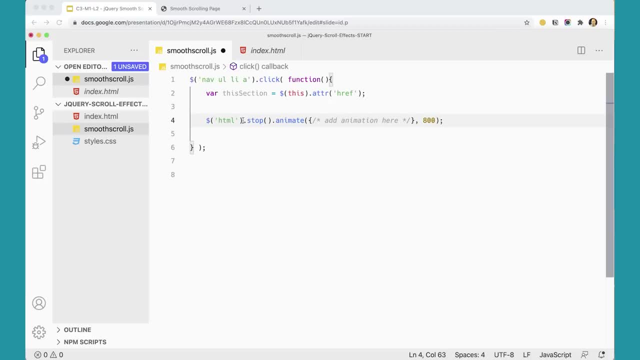 and we'll test this out in a minute. but this is going to actually animate our html and in here we'll use our this section thing to tell us where we're going to animate to, and we'll do that in the next video. so you kind of see how it all comes together. 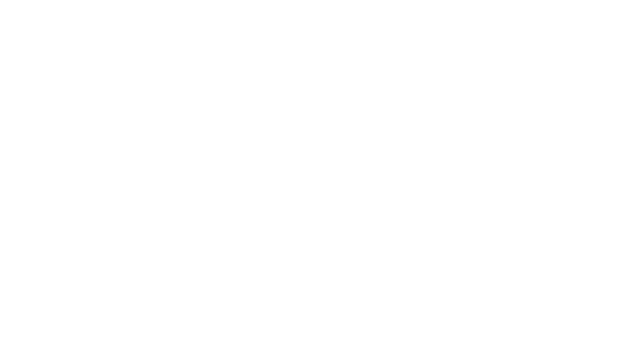 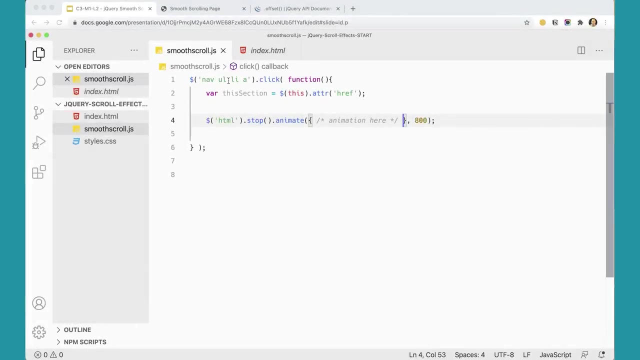 in the previous video, we created a click handler for all the anchor tags and then we got the id of the particular anchor tag that gets clicked on, because you can only click one at one at a time. so what is that? what is the id associated with that, or what's the href associated with that? 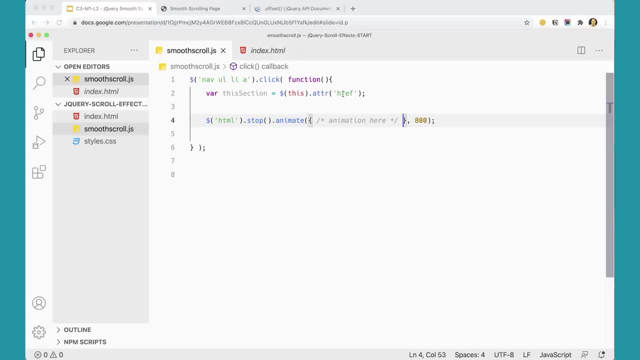 which points to the id of the section down below that we're going to. so it's either going to be pound first or pound second, or pound third or pound fourth or pound fifth. we've already seen that. then we're going to animate the html and I'll show you in a minute what this stop thing does. but 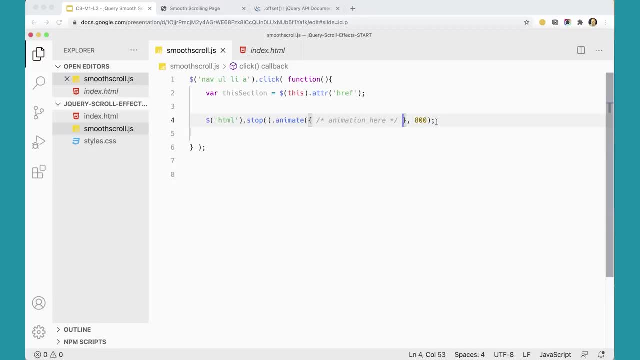 we're going to animate and in here we pass in a key value pair. that is uh, that we're going to actually animate. so what is that key value pair? we're going to animate over 800 milliseconds here. so what is that key value pair? it is the property that we're going to animate is scroll top. 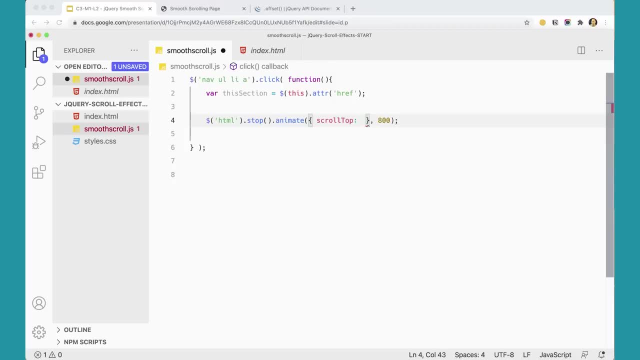 now, what is scroll top? scroll top is an html uh property that you may not be aware of and it returns or sets the position that an element is going to be from the top of the window. so when we click on a particular link, we want to put the corresponding section at the top of. 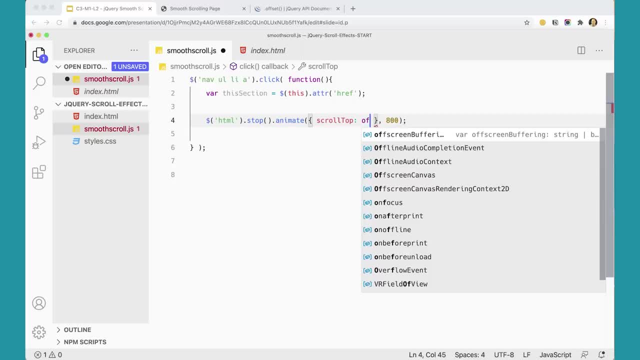 the window. so how are we going to do that? we're going to do it with the offset method. whoops, not sure what happened there. offset method, the offset method, and we want to. we want to offset top. so we'll set it to offset top. oh, and I see why it was upset. usually, when things happen like that, they happen for a reason. 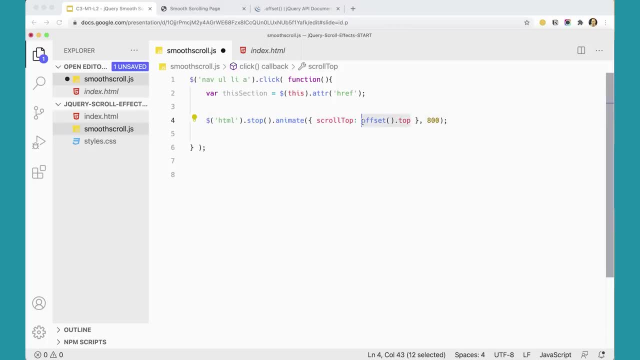 let me do this again. I want to take my variable here, so dollar, sign in parentheses this section and set its offset here. so now we kind of can follow along and move about. so I double click on the 이게 straight check, no problem, and we're going to be able to moves up. 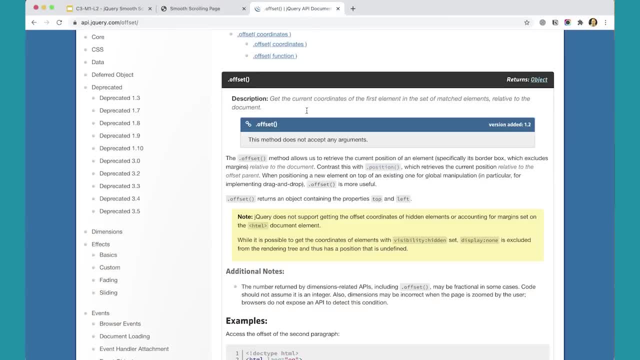 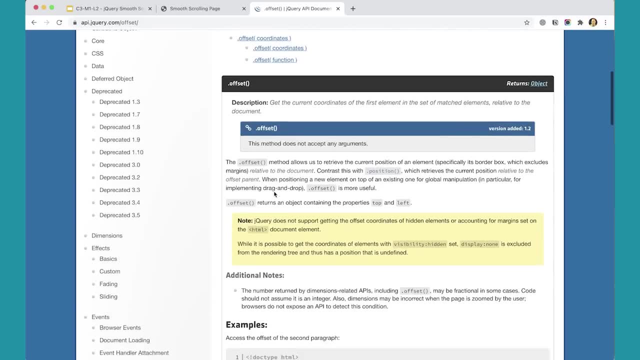 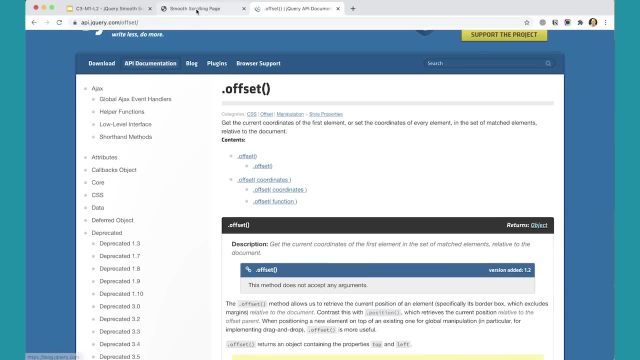 to the top over 800 milliseconds and that will actually animate the page to the top of the window. so if we test this out and if you're wondering what offset is, you can go look it up on the jQuery documentation and see what offset does and how it's used. 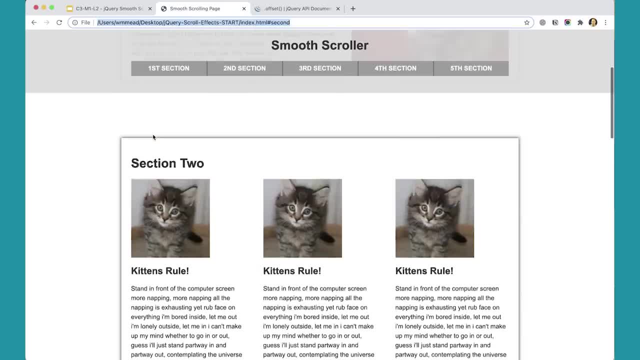 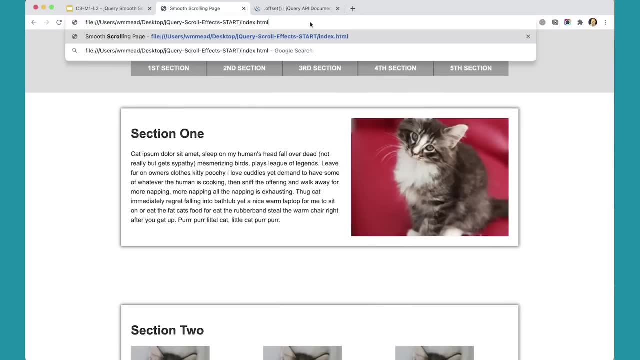 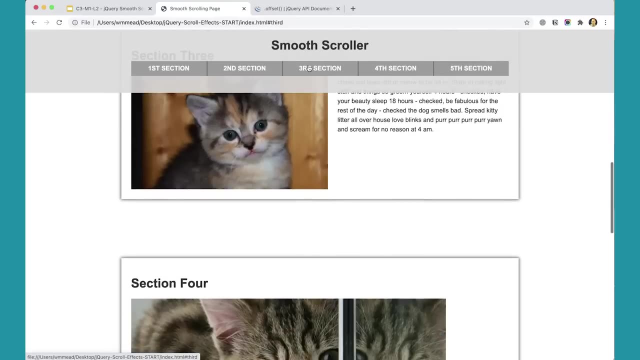 it to or moving it to the top. So let's go ahead and see what happens. if I want to get rid of the pound second from up here and refresh the page, And then if I click second, you can see that it does a smooth scroll right to with that section, going right up to the top of the window. Now 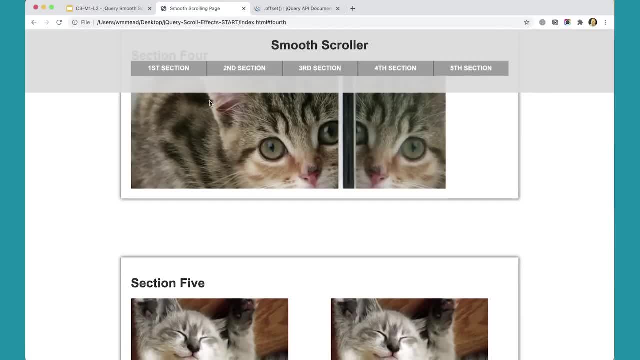 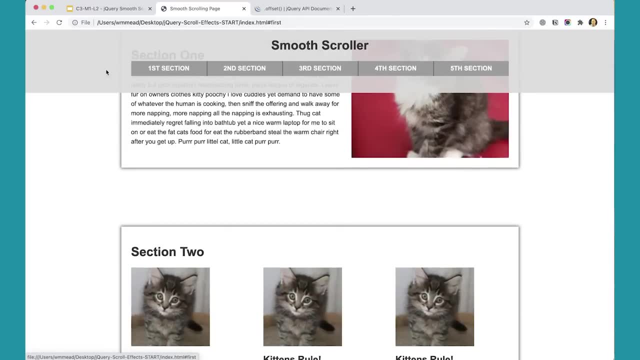 we want it to not go all the way to the top of the window. We want it to stop here, and we'll fix that in a minute, But before we do, what I'd like to point out is what this stop method does. So over here, I'm going to actually set this to a longer period of time. 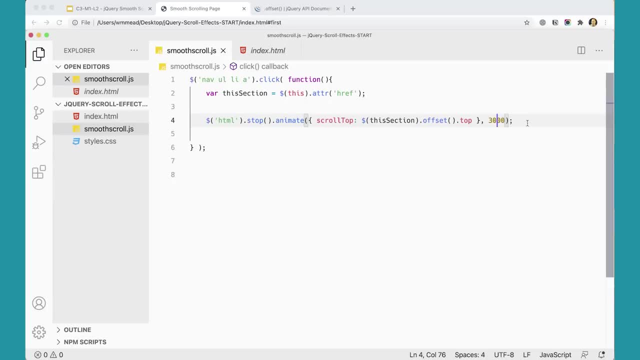 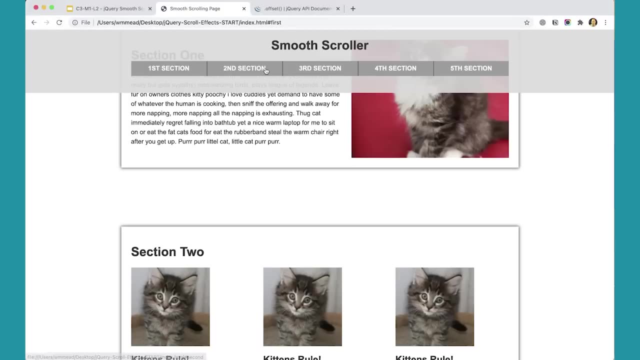 3,000.. It's kind of really long, but I'm going to set it to 3,000.. And if I come back and test this again, you'll notice it'll take a long time to go to the section. three full seconds. 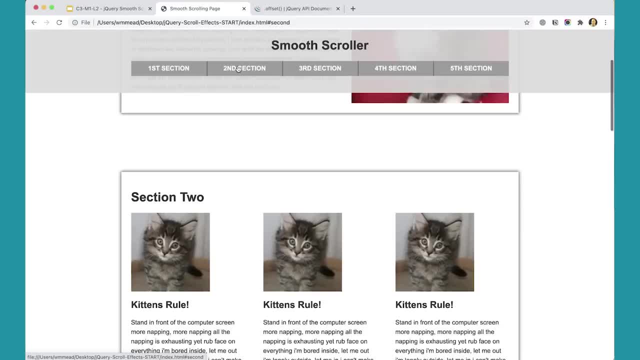 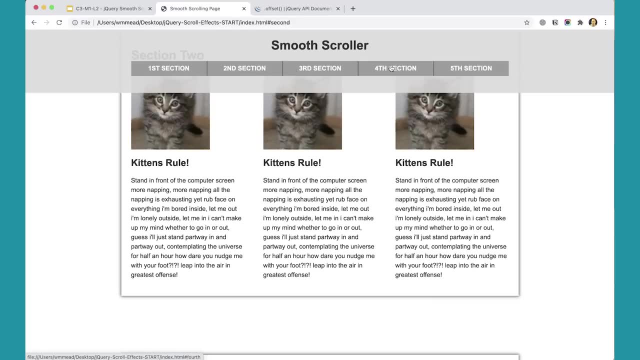 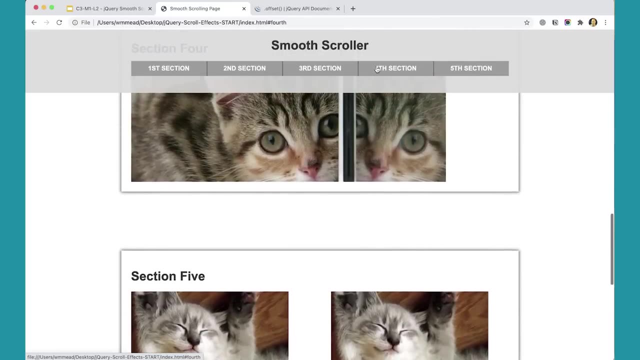 But you'll notice, if I press section one and before it goes there, if I press section two, it'll stop that animation and continue on. It'll continue on to the next one that I've started. So if I press section five it starts, But if I do four it'll actually not finish that first. 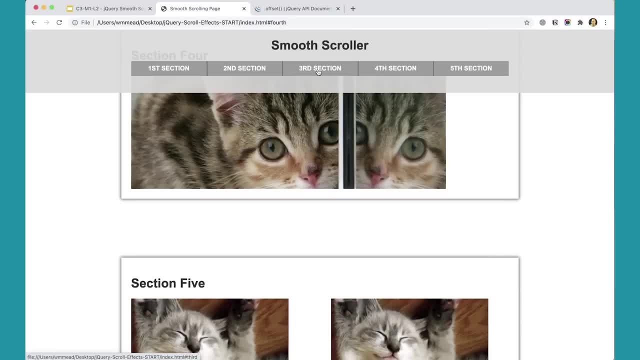 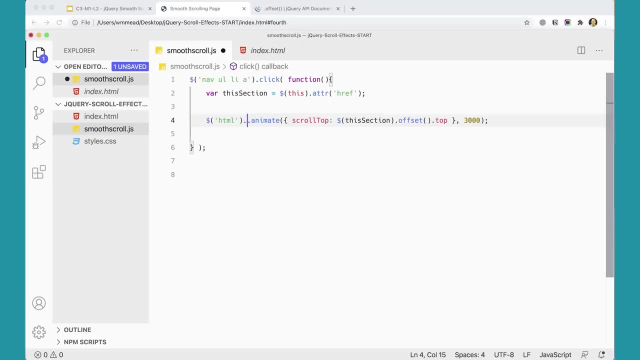 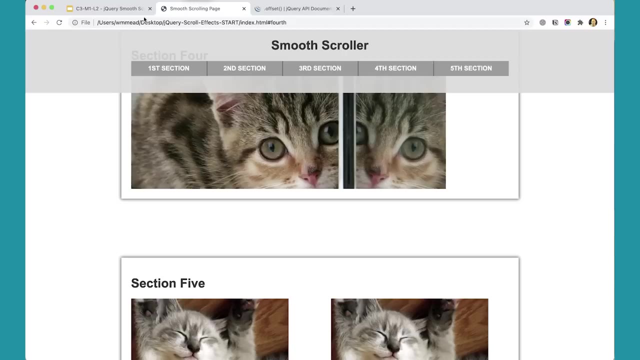 animation and go to the fourth section instead. And that's what this stop method is doing here. If I take stop out, you'll notice that the animations start to stack. So now, if I come back here and go back up to the top of the 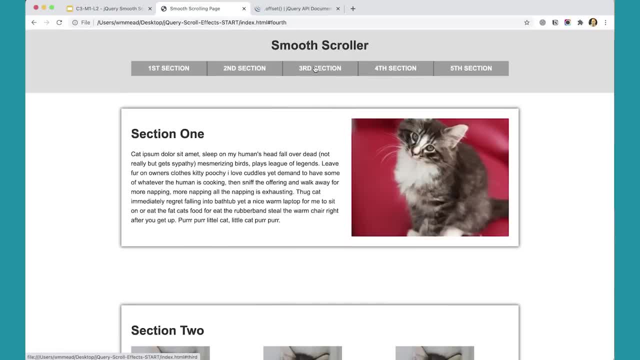 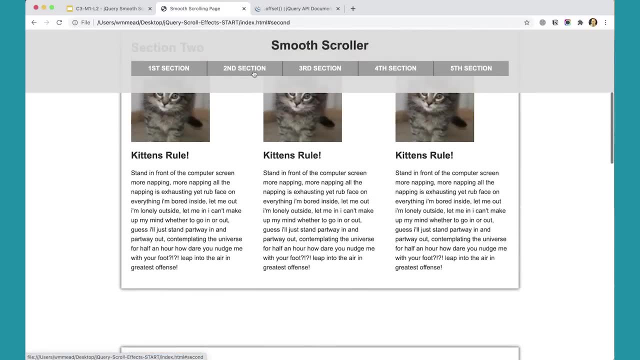 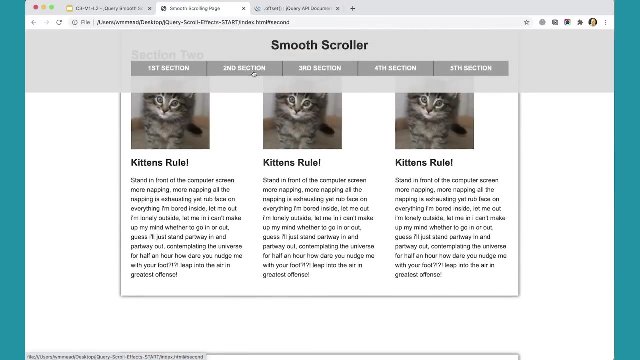 page and click refresh if I press third. well, if I press fourth section and then second section and then fourth section and then second section, you'll notice that the animations stack and it's waiting for each animation to complete before it goes on to the next one, which is not really the 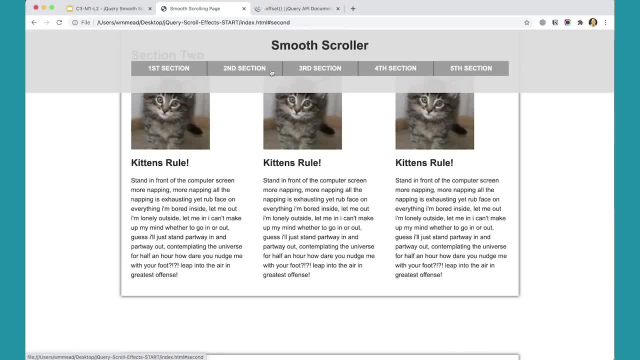 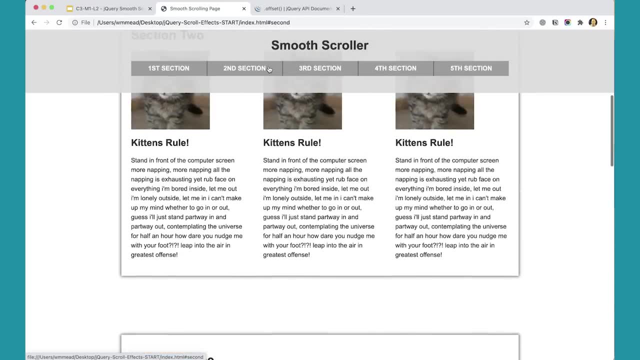 experience that we want to have. So if I wanted to stop that animation, I clicked on fifth section and I've changed my mind and I want to go to the second section. I want it to go there right away, without having to wait for it to go all the way down to the fifth section. 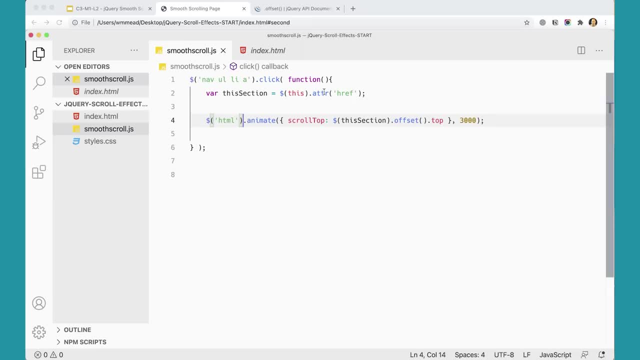 So that's what this stop method is doing for us: dot stop, So it will stop the animation that's running and then animate the thing that we've clicked on next. OK, now the next thing is this: There are two minor things we need to fix. 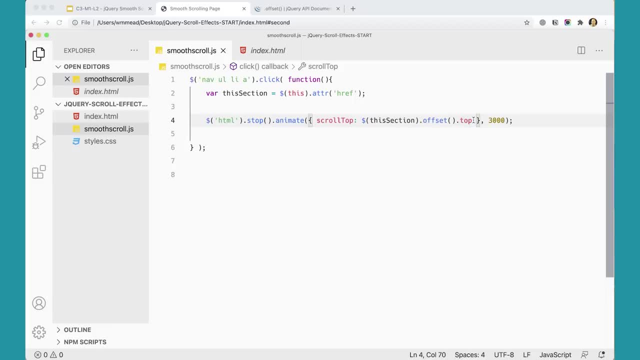 First of all, I really wanted to move to top minus 200. Like so, Because I really don't want to go all the way to the top of the page. So that's one. So now, if I come back here and test this, 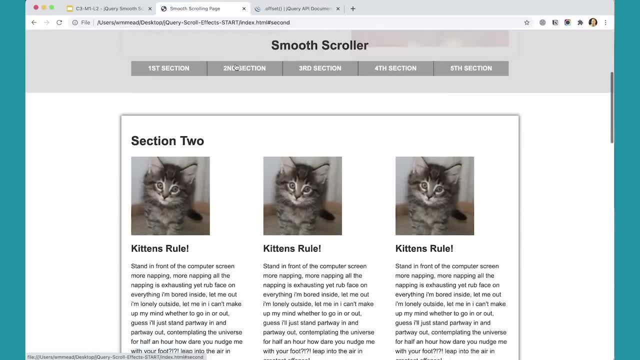 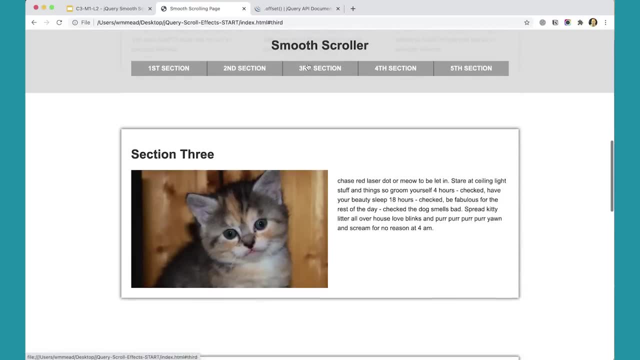 Now, if I click section two, instead of going all the way up to the top of the page, it goes to 200 pixels down from the top of the page, which, you'll remember, we put 200 pixels padding up there, So that's now putting it in the correct place. 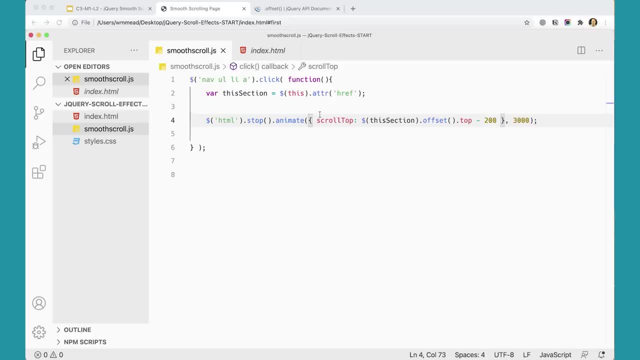 So that helps. So that's one thing. I'm going to put this back to 800 because that animation is so slow. now OK. the other thing is I'm going to put a comma in here and add body. Now, pretty much these days, all the browsers will animate the HTML element and you won't run into a problem with this. 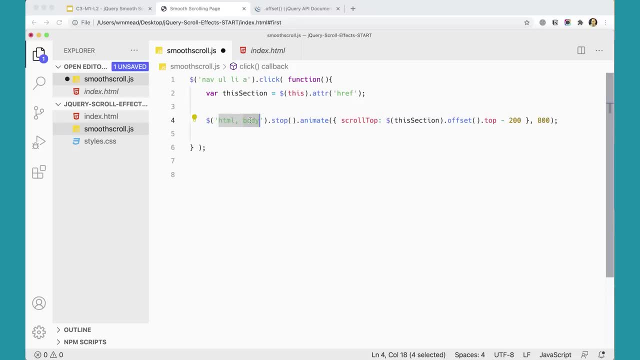 But there have been in the past, certain browsers that won't do that, And so you have to actually put this animation on the body tag instead. Now, in fact, it seems like the most updated versions of Safari and Firefox and Chrome all handle the HTML. 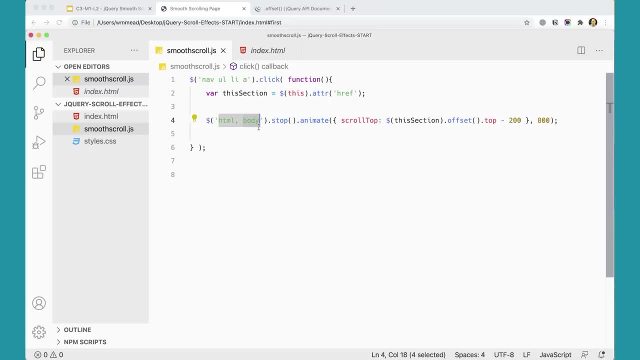 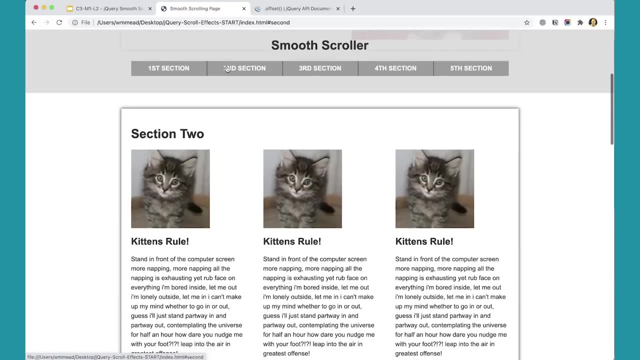 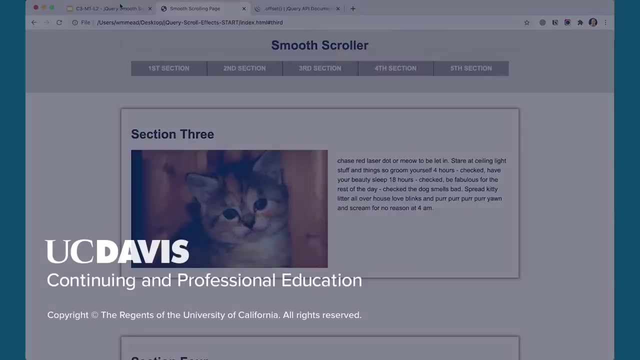 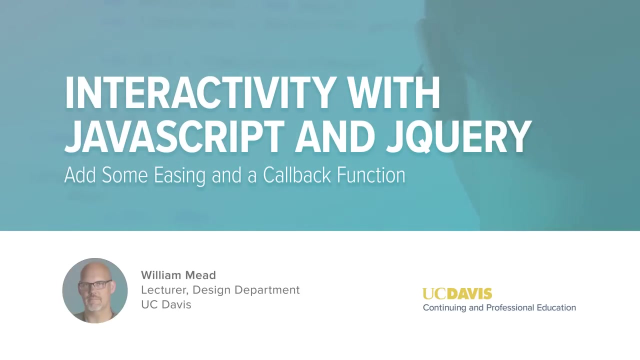 Just fine, But this is kind of just a fallback just in case somebody is using an older browser. Not sure when they actually fix that, so we won't see a difference because of that now, but it's just something to be aware of Going forward. 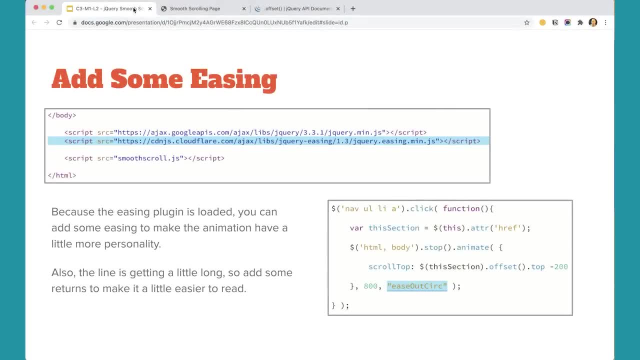 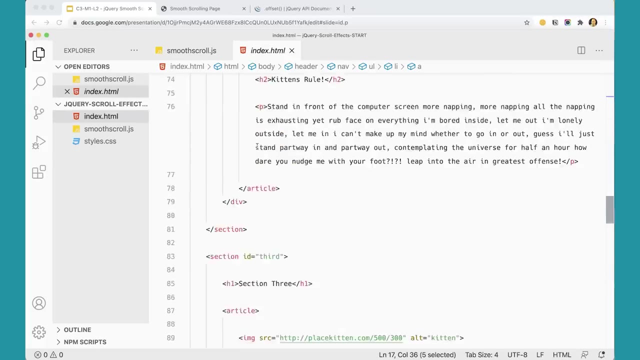 The smooth scroll script is working and that's great. but because we have The easing plug in plugged in, we can give the script a little bit more personality by adding some easing. So let's go ahead and do that. And over here just to verify on our index file here down at the bottom of the page. 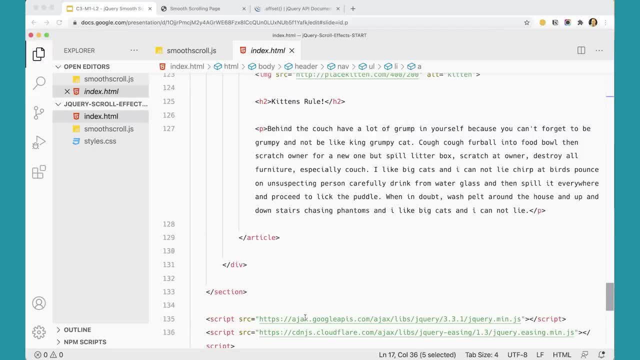 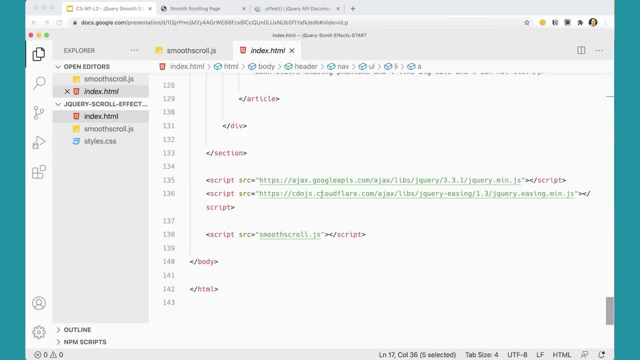 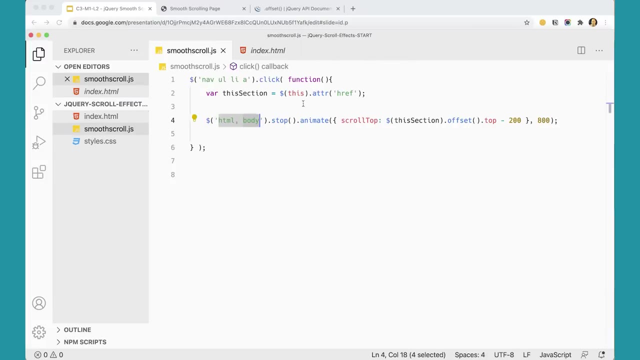 you can see I have the jQuery library loaded and then I have the easing plug in loaded And then my script comes after that. Always, your script has to come after jQuery, the jQuery library and any plugins that you're using. OK, so over here after my 800,. 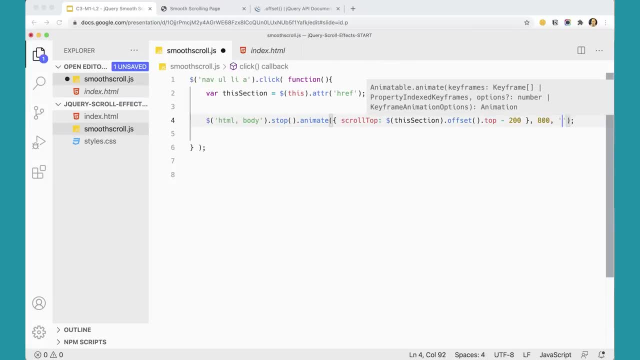 I can add a comma and add an easing, And I used ease out circ as my easing here, which gives us a pretty dramatic set of easing. So if I set that, and then while I'm here I'm just going to, you know. 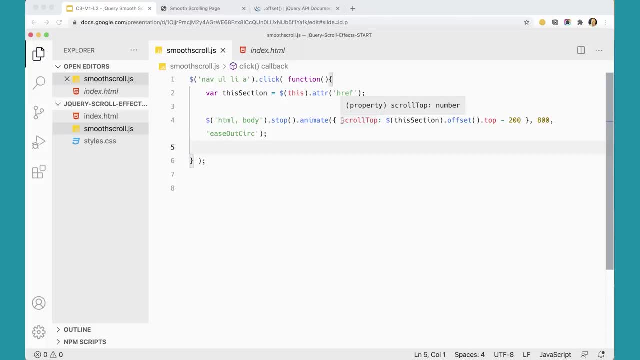 I've got kind of a lot going on in one line here, so I'm going to put a return in here. So that opens and then that closes there. I'm going to move that down like so There we go, Ease out circ. 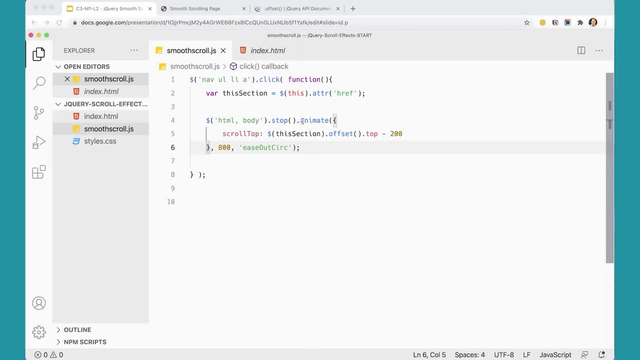 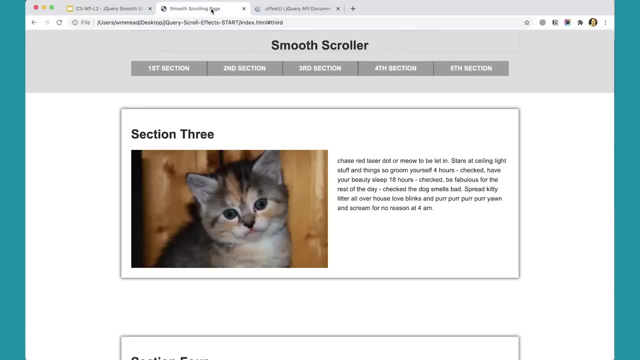 I think that looks a little bit better, a little bit easier to read. So animate, we animate this over 800 milliseconds and we're going to use ease out circ. Let's go take a look and see how it looks. So now it's got a nice sort of slightly snappier feel. going to the sections: 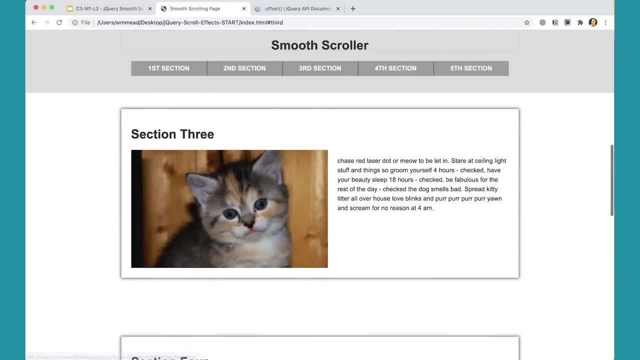 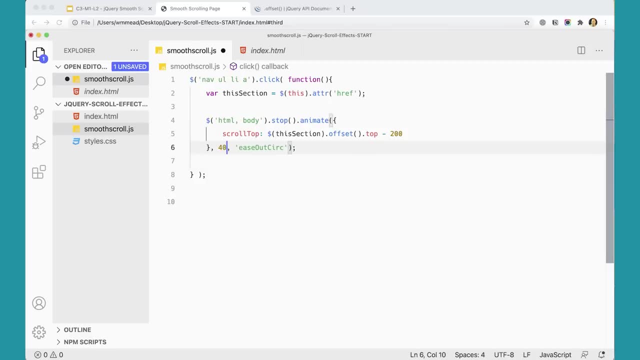 And if it's still going too slowly for you, you could reduce the time further. Come over here and set this to: instead of 800, set it to- I don't know- 400.. We'll cut it in half and see what happens. 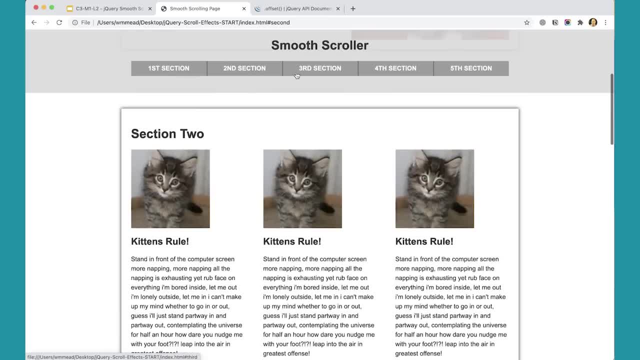 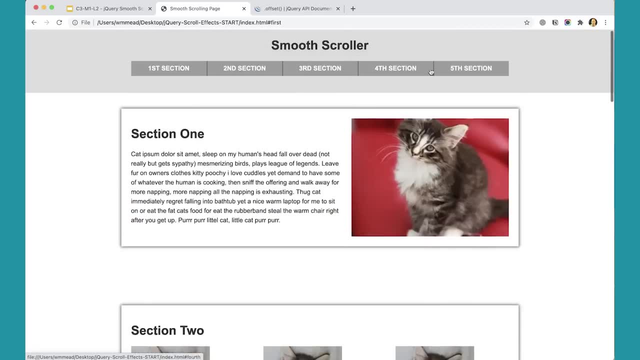 And you have to kind of find the right setting that you think feels good. This feels, you know, very snappy, It goes there very quickly, But does it still give you kind of the sense that you're traveling to that part of the page? 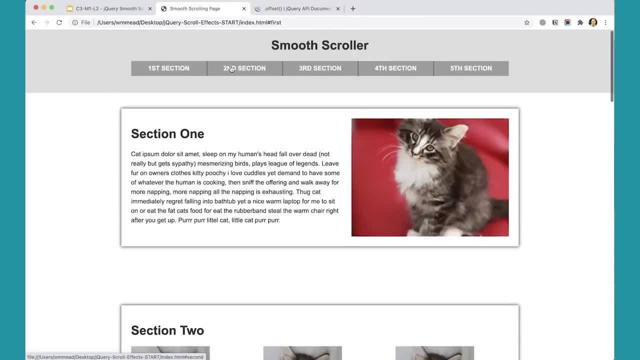 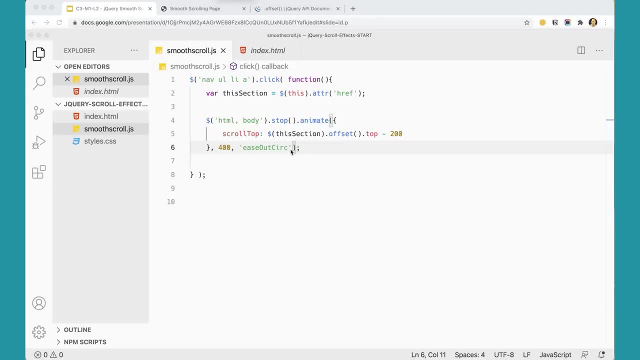 Yeah, it does, So that's kind of nice. Maybe I'll leave it like that. This is all working, and I could leave the script like this. It's certainly functioning, but I want to do a little bit more with it, And what I want to do is actually change the highlighting on these links. 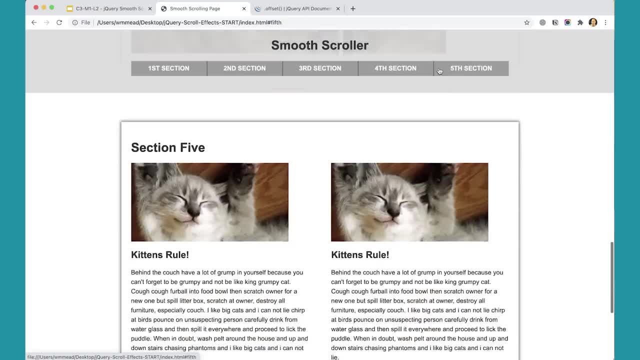 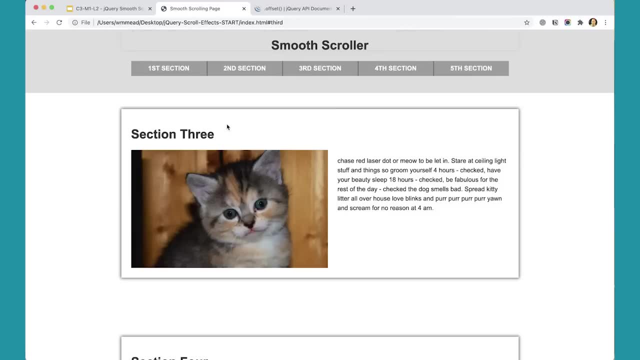 to indicate which link I've I'm actually on when I get to that section. So up here this becomes an indicator of which section I'm looking at, along with sort of the label on that section. So I'm going to do that by adding a callback function in here. 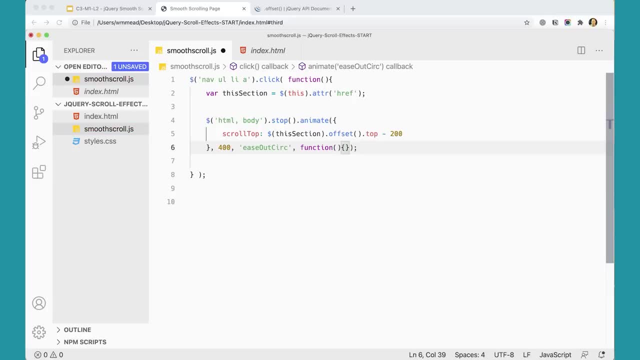 Function. So, after the animation completes, I'm going to run a function in here. In this callback function I'm going to add an alert And in the alert I'm going to add a function, And in the alert I'm going to add a function. 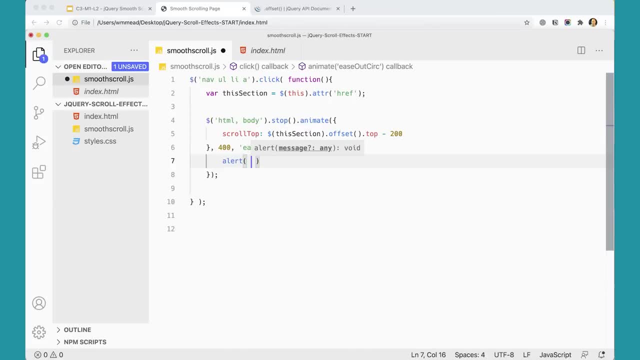 And in the alert I'm going to add a function And in the alert I'm going to actually alert out the offset so that you can see how far from the top of a page the element actually is, how far off the top of the window. 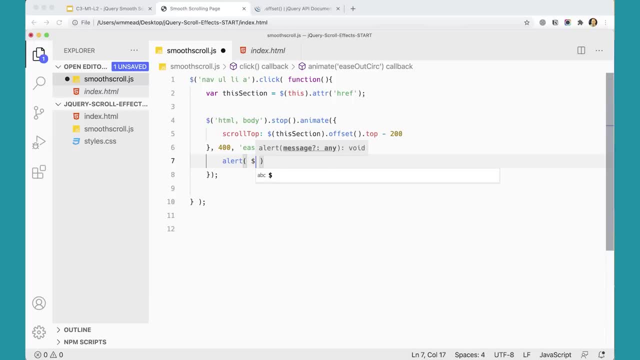 really is what it is. So I'm going to use my jQuery object to go get the window and see what it's offset. Is it offset? I think it's like that offset. If I've done that right, There we go. 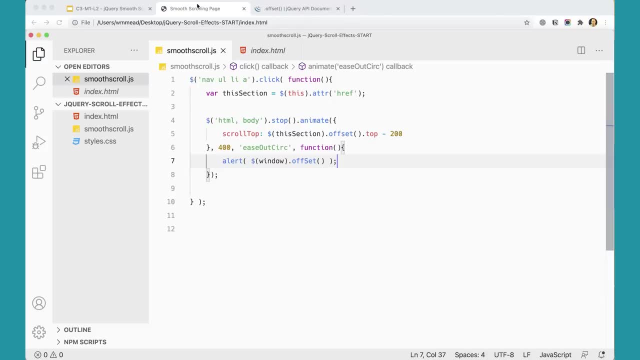 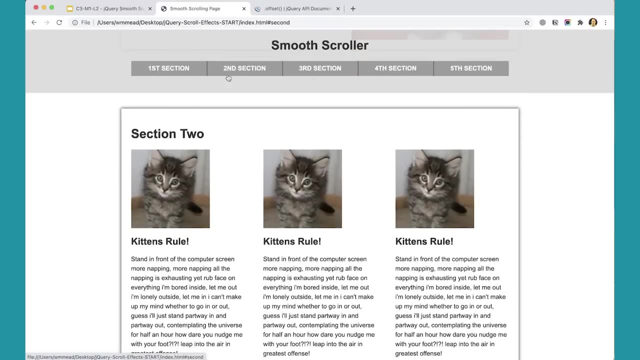 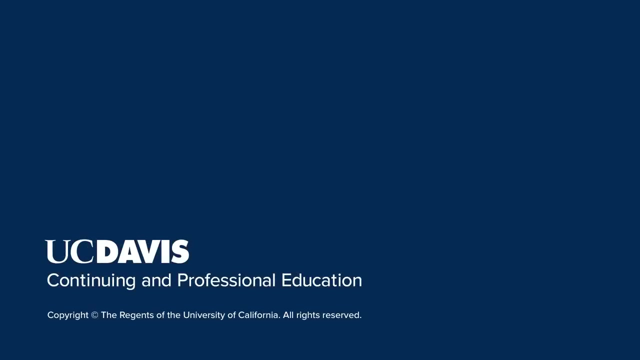 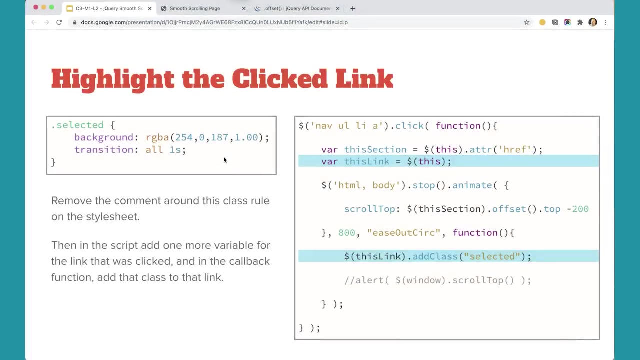 Let's see if I did that right. I think I did. I come back here, refresh the page, click second, and I did something wrong. there On the style sheet is a rule selected and I might have it commented out. Let's go over and see here. 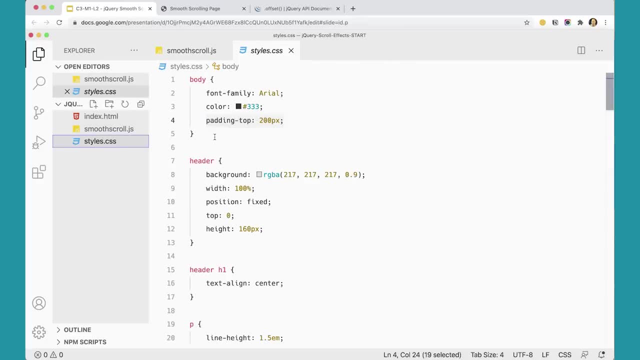 So if we do, we need to uncomment it out. So if we go to styles, go down here and it's not commented out, All right, good. So I've got selected here and it's set to a color and it's got a transition, a one-second transition for transitioning that class. 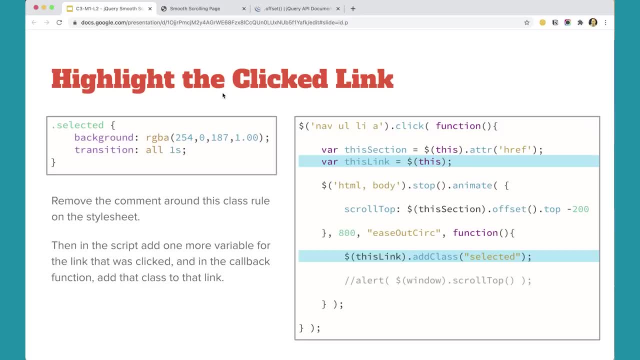 And what we're going to do is we're going to change the link that we clicked on. We're going to add the class selected to it, So I need to add a variable, this link, and it's just this, the link that I clicked, the item that I clicked. 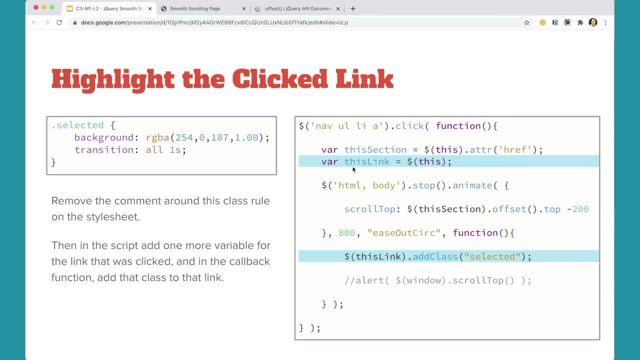 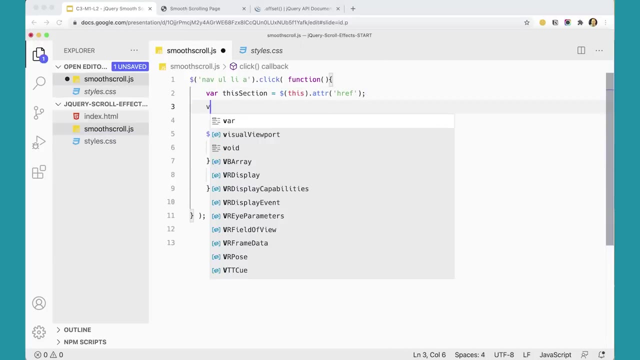 And I could just use this down here, but I think it's a little bit helpful to have the variable name. So this link is just the thing that I've clicked. It's this, So let's go ahead and add that On our smooth scroll script. here up at the top, I'm going to add a variable bar. this link equals dollar sign. this: 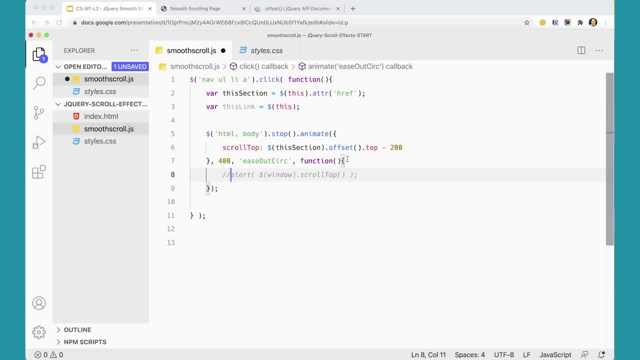 And down here. we don't really need this alert anymore. I'm just going to comment it out. I'm going to leave it there in case you want to refer to it. That scroll top stuff can be a little bit confusing, So sometimes it's helpful to have that in there just to remind yourself what the heck scroll top is. 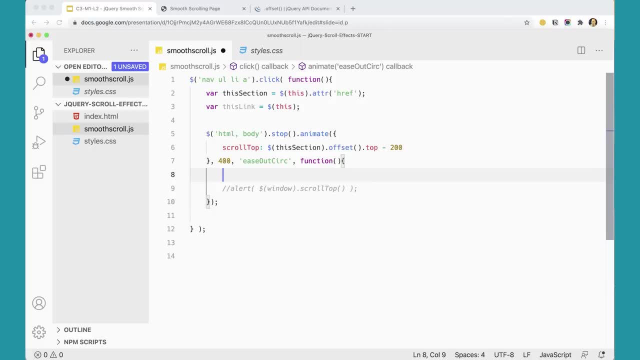 And how that's actually working. All right. So now I'm going to say this: link dot ATTR. Am I using class name? I forget what I put over there. I'm using add class. Okay, We'll use that method. You could also use the ATTR method, but I'm going to just use add class. 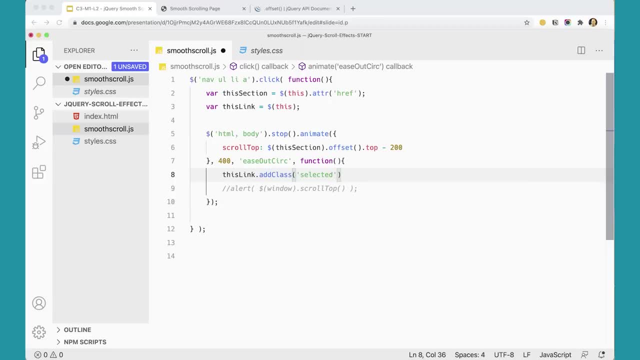 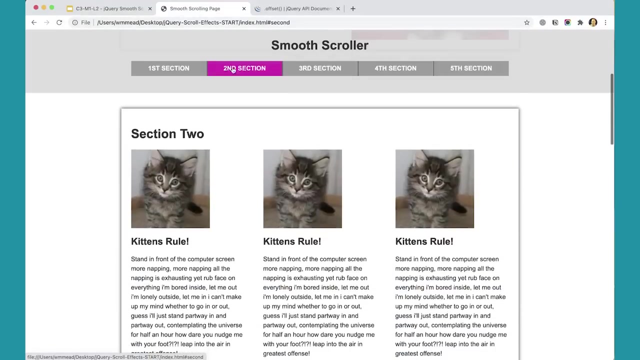 Selected. Now there's one small problem here, in that this will work the first time you click on a link, but it won't work every time. So we'll see here as we use this. When I click second, it'll add the class. 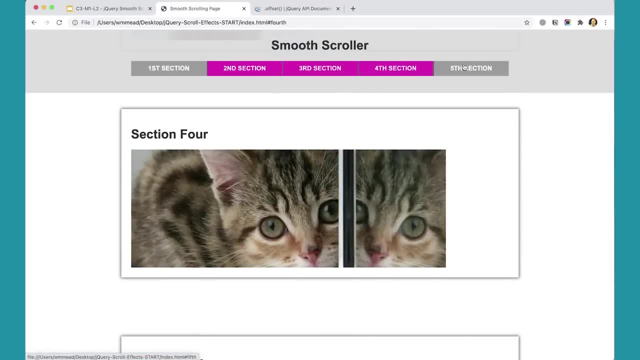 And then when I click third, it'll add the class, And when I click fourth, it'll add the class. So it's working. But what I really wanted to do is remove the class from these and then just put it on the one that I've clicked. 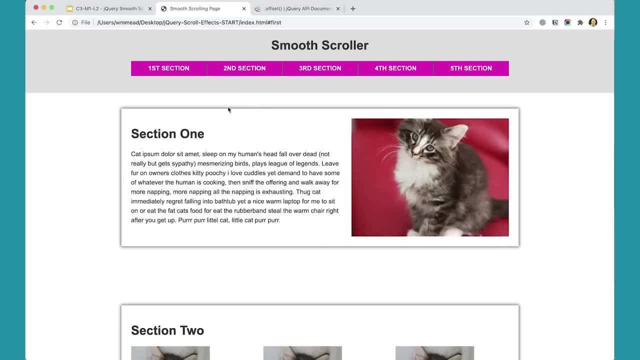 So they don't Just all turn pink, Although you could have an interface that shows well, which ones have you clicked on, And it would work for that, But I really wanted to just highlight the one that I've actually clicked on. 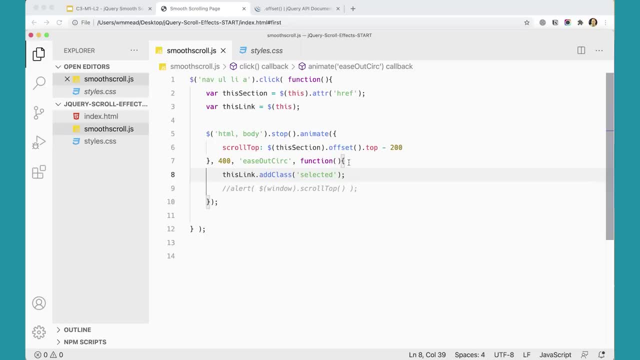 So I'm going to go back to my script and I'm just going to modify just a little bit here by saying: Use my jQuery object to go in here and get all those anchor tags Nav, U-L-L-I-A. And here I'm going to use: 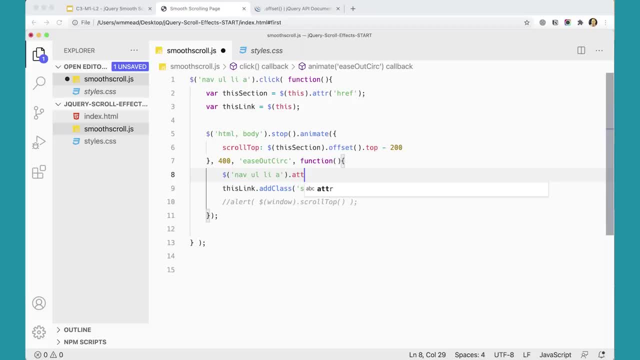 A-T-T-R Or. I don't think I want to do that, I think I want to do something else. I want to use actually Remove A-T-T-R. Remove attribute Class. I'm going to remove the class attribute. 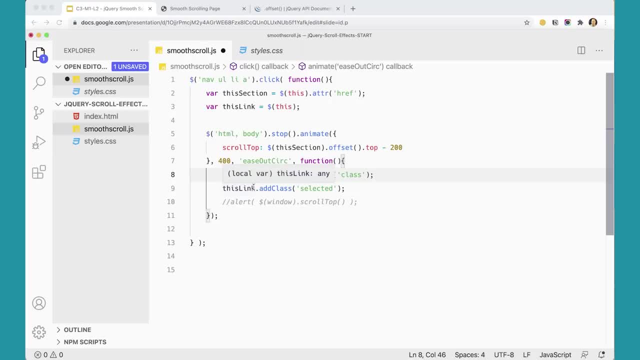 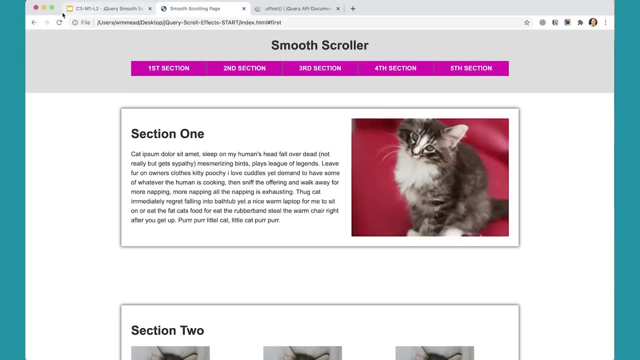 So that removes the class attribute from all of them And then just adds it to the one that I've clicked on. Let's see if that works. Come back here. Refresh the page. Now, when I click on that it adds the class there. 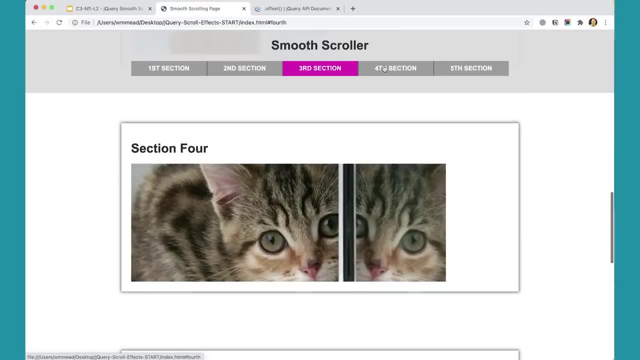 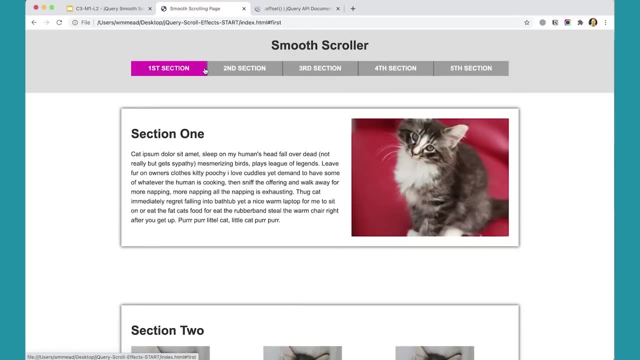 It removes the class from all of them and then adds it to the one that I clicked on, So that's working great. Now you could go back at the beginning when the page loads and just add: selected to the class of this element, of this first one here. 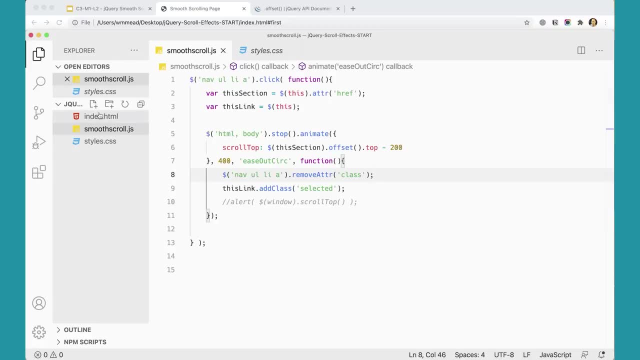 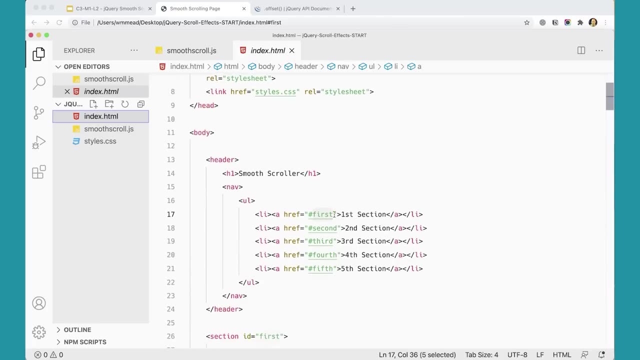 Let's do that Just so that when the page loads We're obviously Going to be up at the top of the page. So we might as well have Class Oops, Class equals- quotes selected On that first link In the navigation. 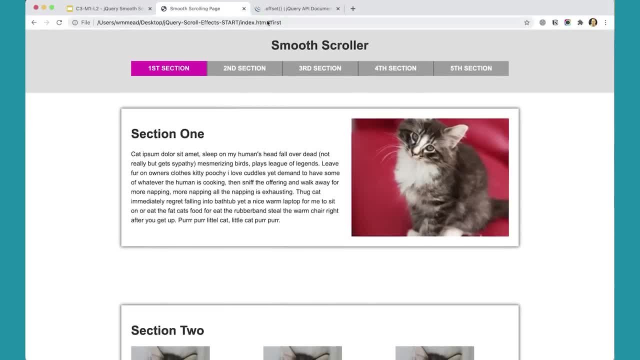 So that now, when you load the page from the start And get rid of this stuff here- Press return- That comes up select, because that's what we're showing. We're showing section One and then we'll go to section two and it'll turn off all of them and then add it there. 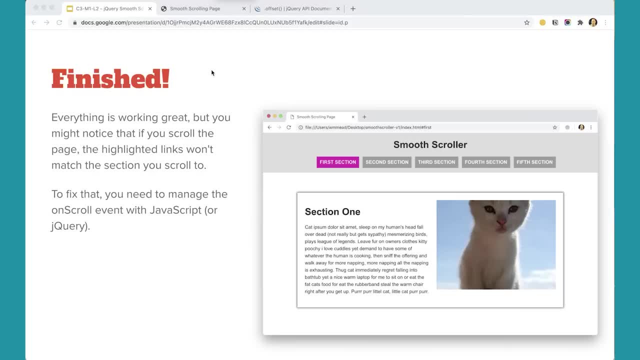 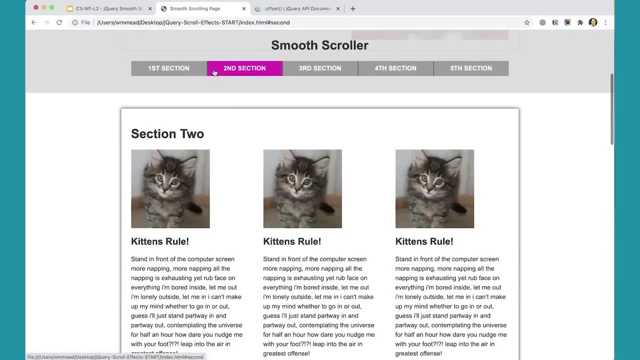 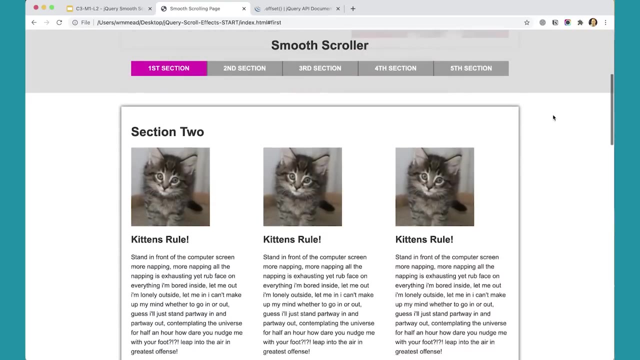 And that's working great, And with that, this part of this script is finished. We have a script where we can click on these, and it will animate to that section and highlight the correct section. One thing you'll notice, though, is that if you scroll the page, it doesn't change these: 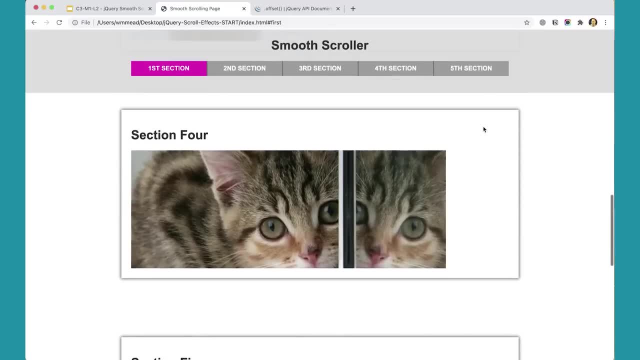 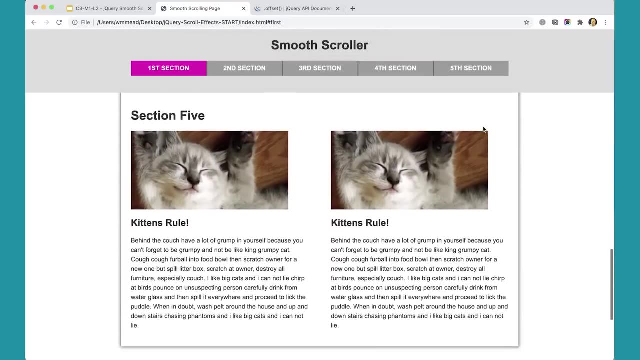 What's highlighted Up here And to do that, we really need to manage this scroll scroll event so that we can handle what happens as we scroll the page and move from one section to another. So we're going to deal with that in the next lesson. 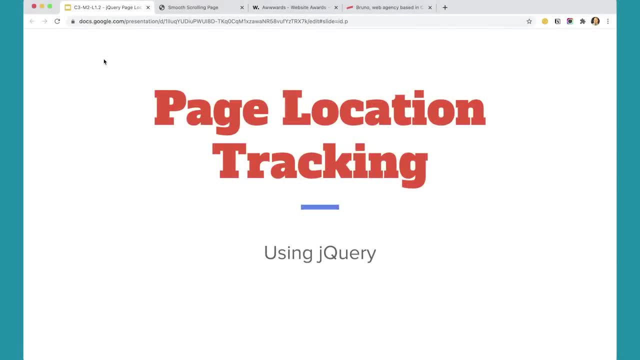 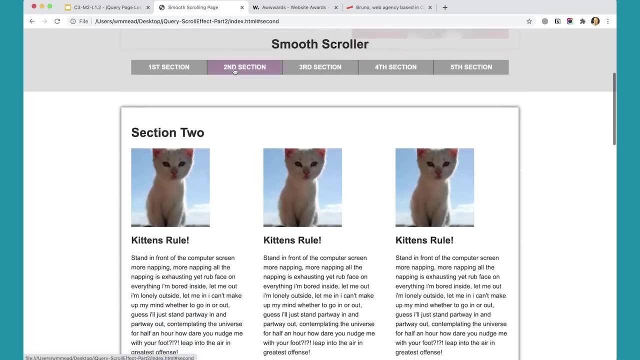 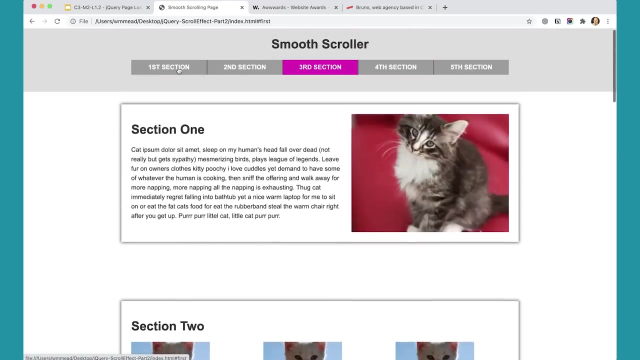 Page location tracking using jQuery. In this lesson we're Going to take the files that we already started here And this script is working so that if I click on the section, it goes to the correct section and it highlights the correct menu item up here. 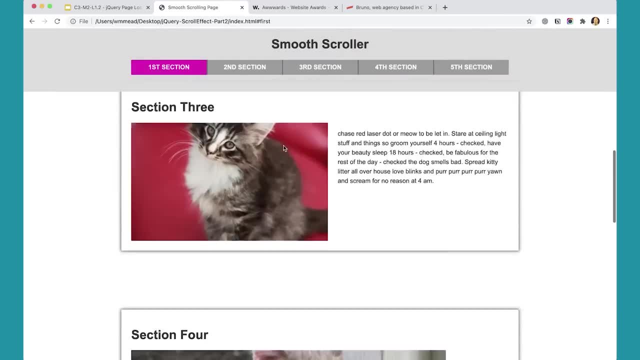 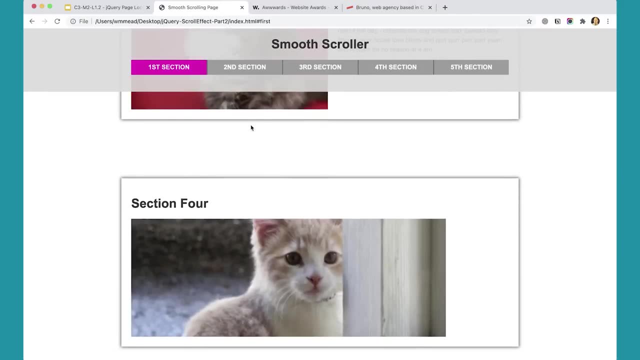 But what it does not do is, if I scroll down the page, it doesn't change the highlighting to demonstrate the section that I'm looking at here. And this may seem like a little thing, a minor detail, and I suppose that it is in this page. 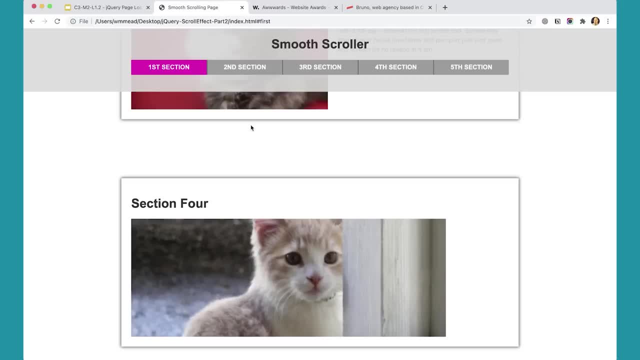 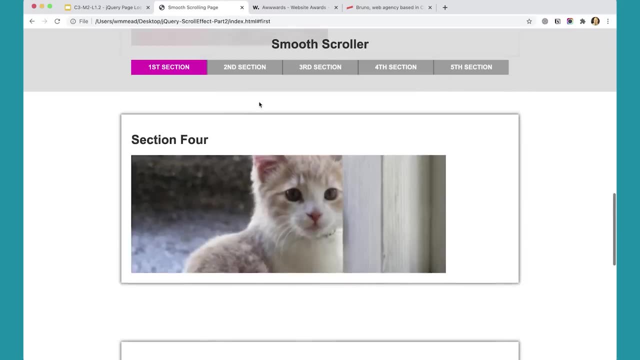 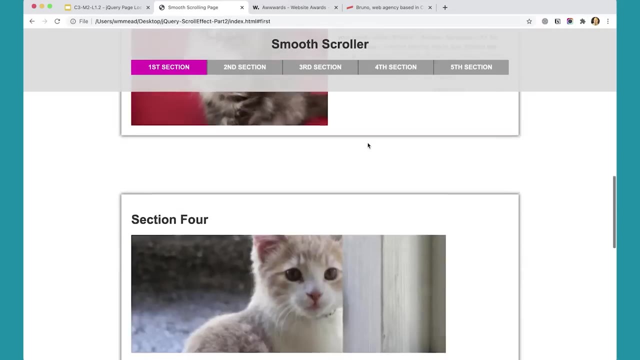 And we're going to work on a script to fix this, And it may seem that the script we're creating is awfully complicated to fix such a small thing, But what's really cool is the script that we're going to write that will allow us to change the highlighting based on where we are on the page is capturing the scroll event. 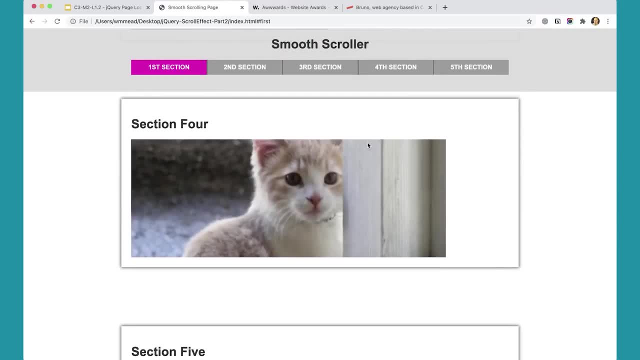 And working with scroll scripts can be challenging because there are some, there's some difficulties that you have to deal with, But The really cool thing Is really cool thing is that if we could get these things to highlight, we could do anything on the 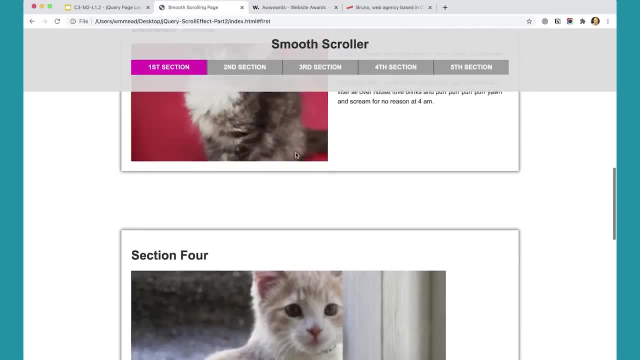 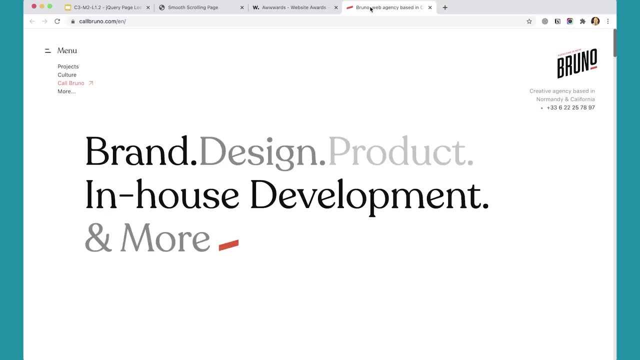 page based on where we are scrolled on the page And if you think about that for a second and go look at some of the interesting websites that are out there. So, for example, I have one pulled up here, this website here, And as I scroll down, different things are happening based on whether. 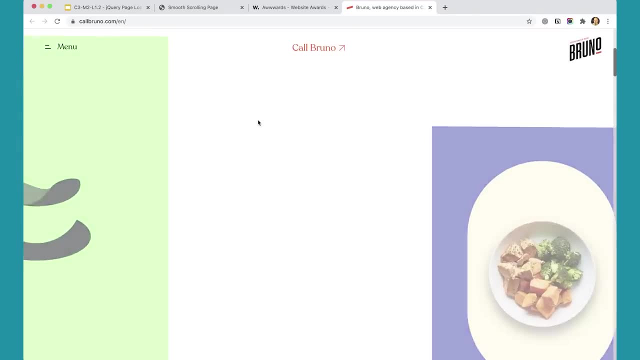 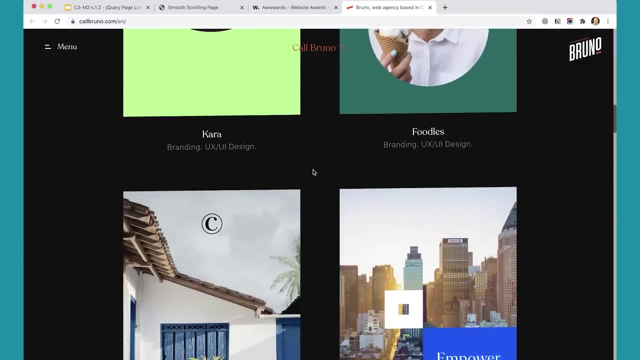 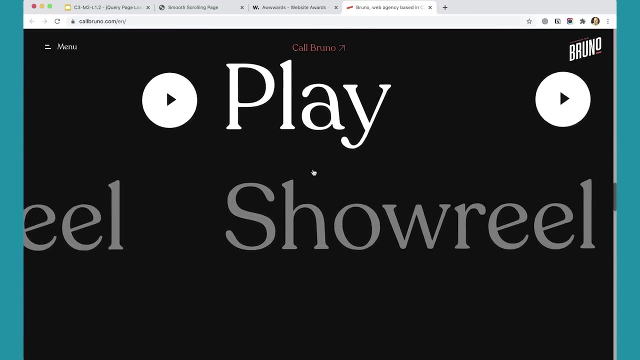 I'm scrolling, Scroll down, this happens. Scroll up, those go back out. So this is capturing a scroll event and doing something on the page based on whether or not I'm scrolling. So I scroll down the page. here That animation plays differently while I'm scrolling up or scrolling down. 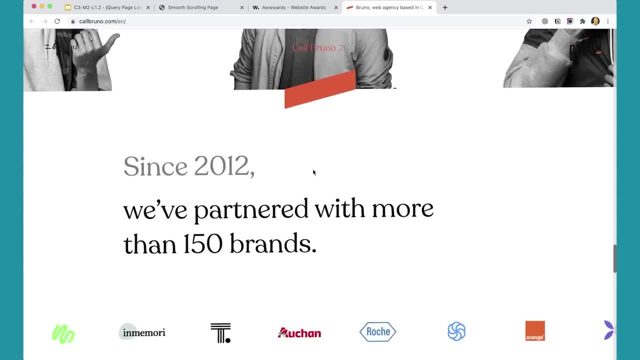 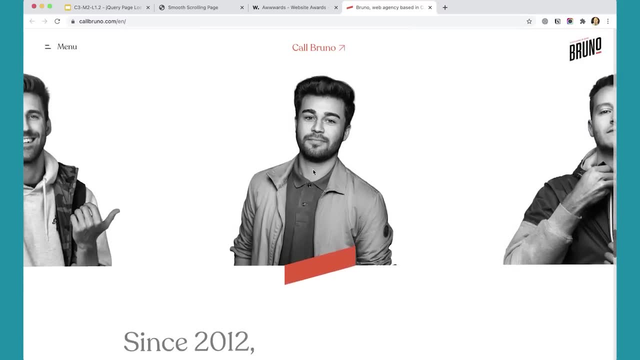 It's affected by the scroll, And down here there's another one, So that just switched to white, which switched based on where I was scrolling. If I scroll up, it'll switch to black or dark gray And when I get down here, this set of icons. 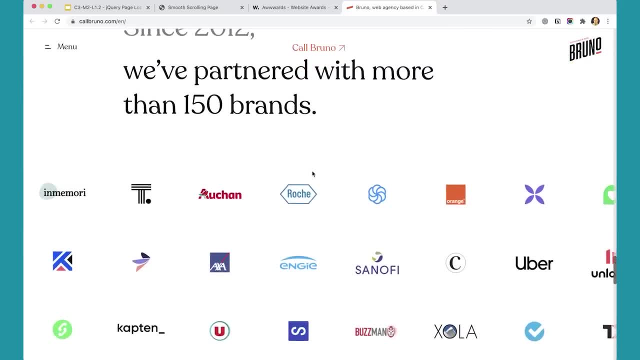 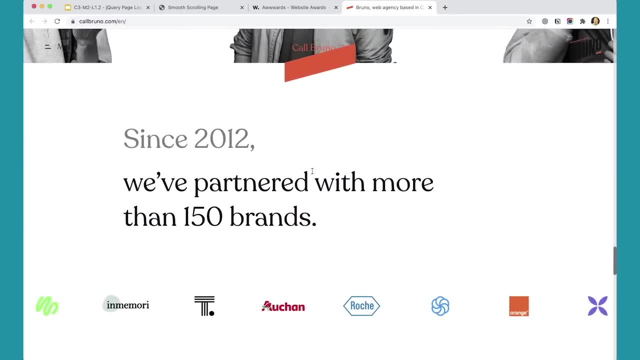 is scrolling, is moving based on whether I'm scrolling or not. So if we want to be able to do any of these types of effects, you need to capture the scroll event and you need to be able to do things with that scroll event when you capture it, And that can be a little bit challenging. 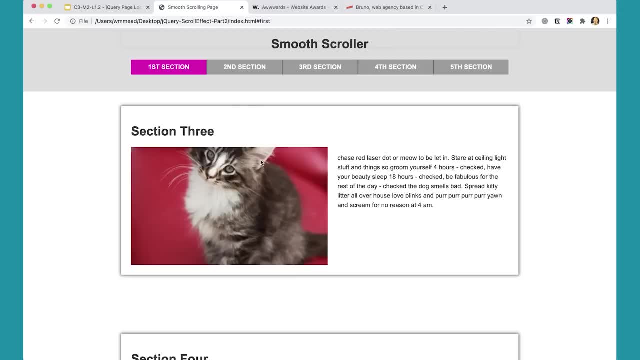 And we'll get into why in just a minute here. But for right now, for this script, all we're going to do is change the highlighting on these links, which seems like a very minor thing. But just keep in mind that when we're done with this script, 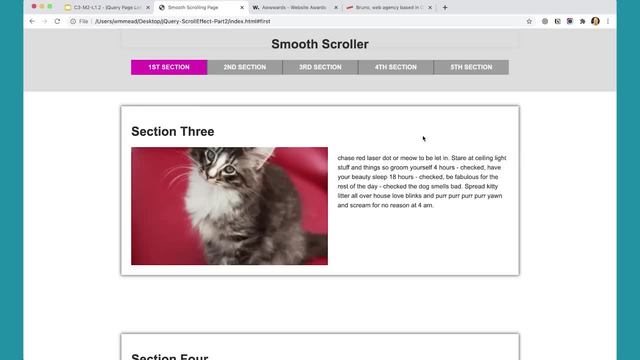 we will have a script that you could use on lots of web pages to track where you are on the page and do lots of different animations or cool effects or other kinds of things based on where you are on the page. So that's pretty exciting. By the way, I should add that I don't know. 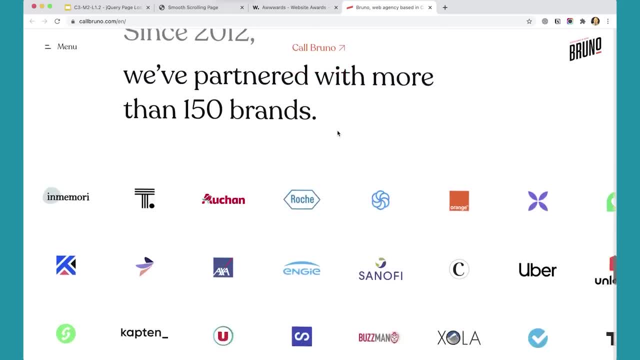 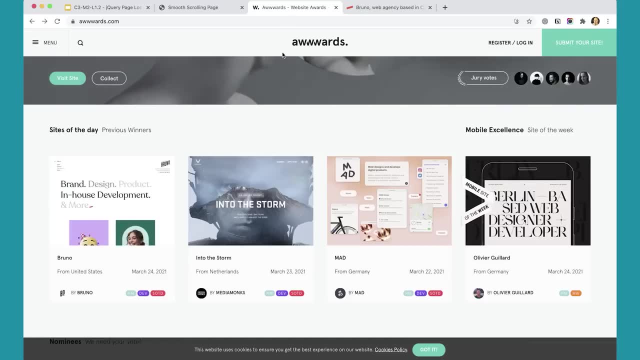 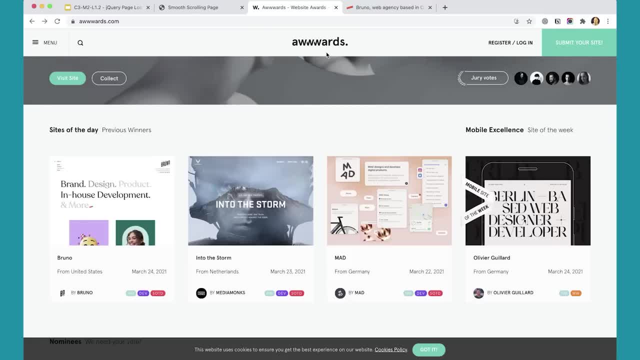 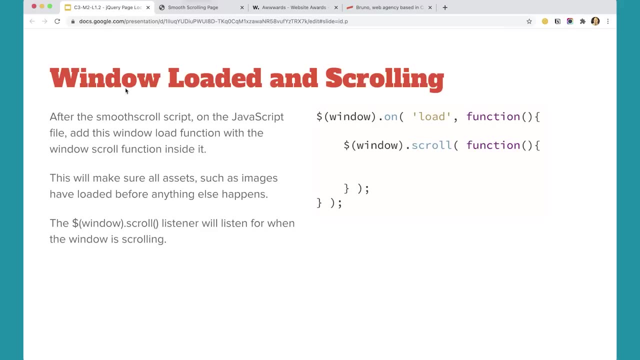 come to- I think I've pointed out in previous lessons- if you want to see some interesting interactions that people have created on the web. they often get posted here, So this is a good place to come to get inspiration about different kinds of things that you can do. Okay, let's get. 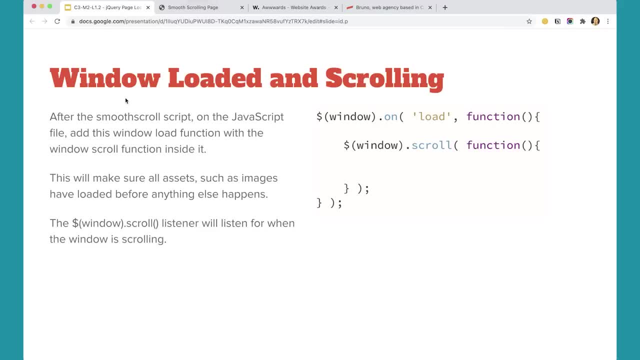 started with our script And we're going to work with the same files that we just completed. You don't need to change anything. We're going to start with the same files that we just completed. You don't need to change anything on them. We're just going to continue to work on the JavaScript. 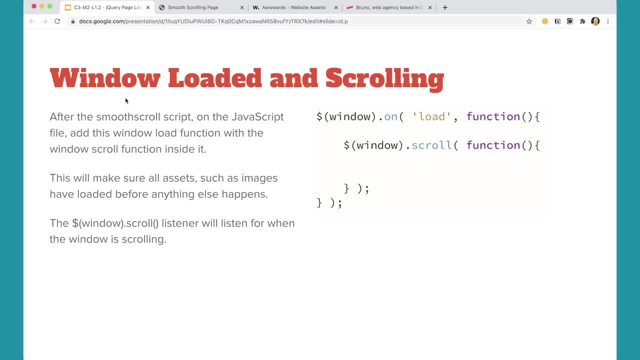 file in that folder And we're going to start by adding an event handler that waits for the whole page to be loaded. Again, we don't want anything to happen until the whole page has loaded with all the images and everything else, And then we're going to capture the actual scroll with. 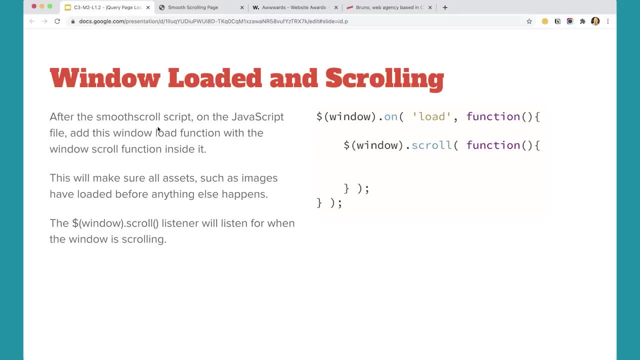 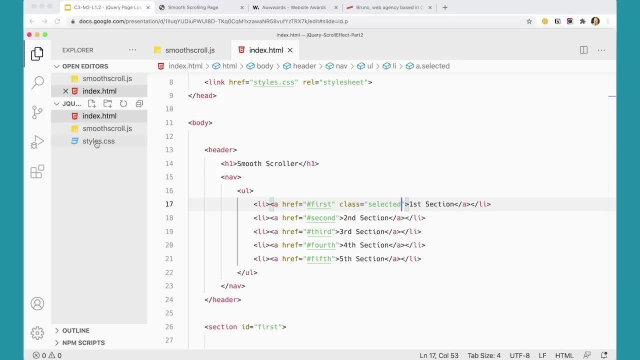 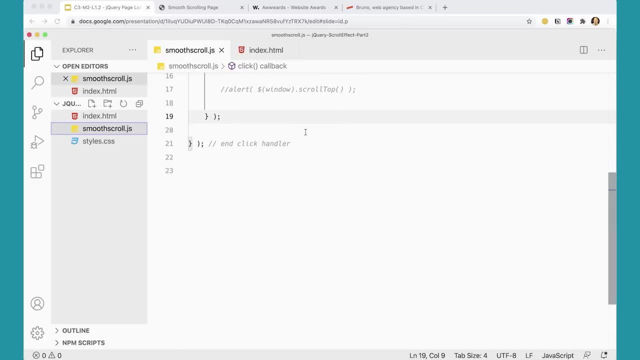 an event handler for capturing scroll using jQuery. So let's go ahead and add this to our script here. So over here on my smooth scroll page here, I'm just going to go down here. So we've got this script is handling the smooth scroll And I'm going to click after that And I'm going to 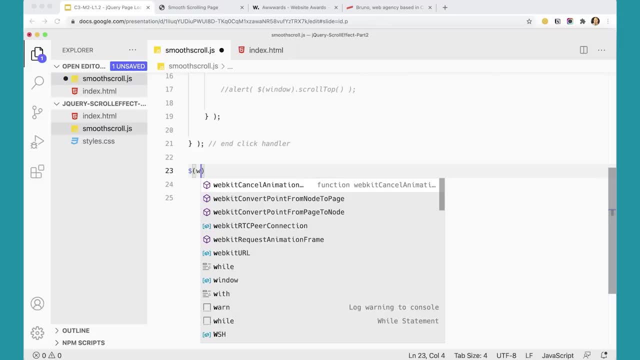 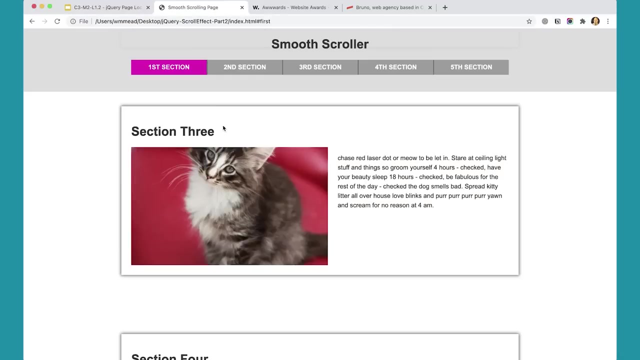 add a jQuery object for window, the window object dot on load. we're going to run a function And this function runs when all of the content of the page is loaded, And in this case, that's important because we're going to be. one of the things we need to keep track of is how tall each of these. 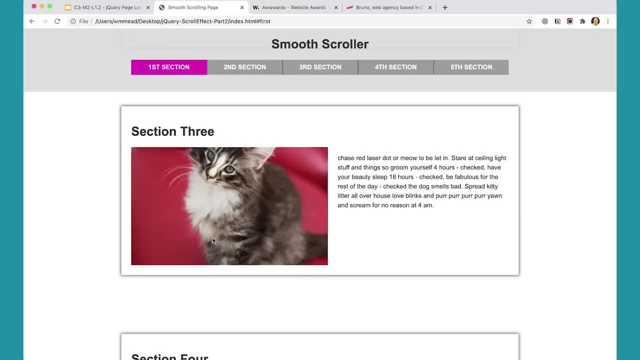 sections are. Well, how tall this section is has something to do with how large this picture is. If this picture wasn't here, this section would take up less space because it would end here, So it wouldn't be that tall. If I want to track which section is on the screen, I need to know how big the 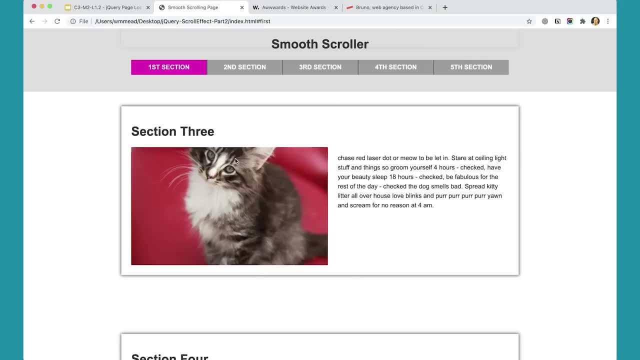 section is For me to know how big the section is, all of the content has to be loaded, including images. or, if I had videos or other content, it all has to be loaded Before I say, well, how tall are you. and I need to know how tall you are so I can know whether this sections on the page or 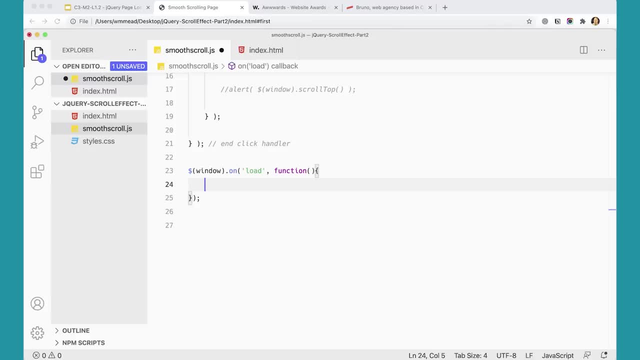 not, So that's why I need to make sure I put everything inside this window on load callback here, to make sure that I'm capturing when the window loads so that everything I do is inside of there. and then I'm going to next add the jQuery object for windowscroll. 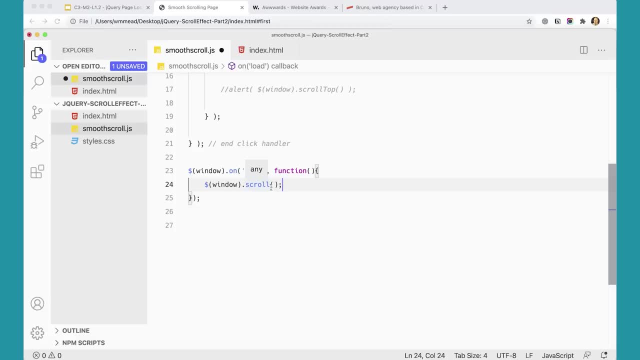 and this will tell us, And this event will tell us- if the page is scrolling at all. And, as with up here our click handler, we're going to pass in a function that's going to run when the page scrolls, So this function runs when the page scrolls. 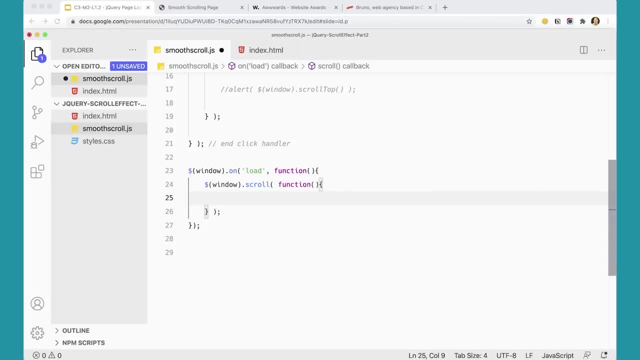 And that's where we're going to put. our script is inside here as the page scrolls And I could just for right now I could just do not alert, but I could do consolelog. You don't want to do alert because you'll get a ton of alerts scrolling. 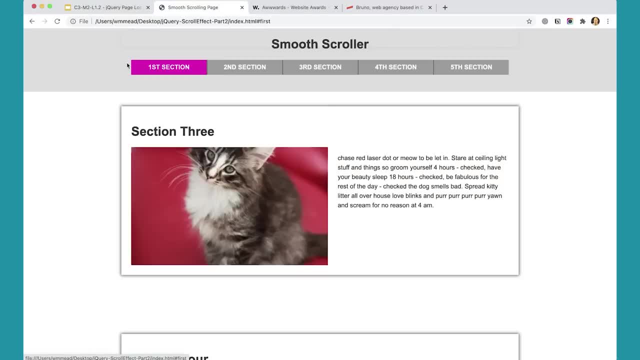 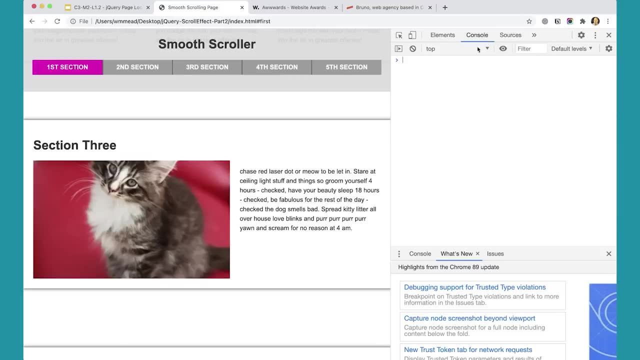 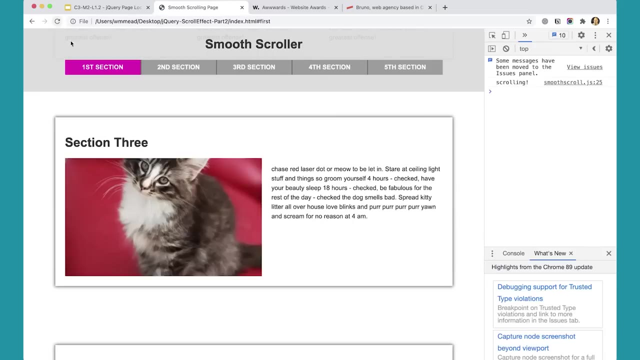 And save that. And if I come back to my page now and choose my inspector over here, turn on my console, Make that a little bit nicer. I'm going to refresh the page And as I move it you'll see this event is firing. 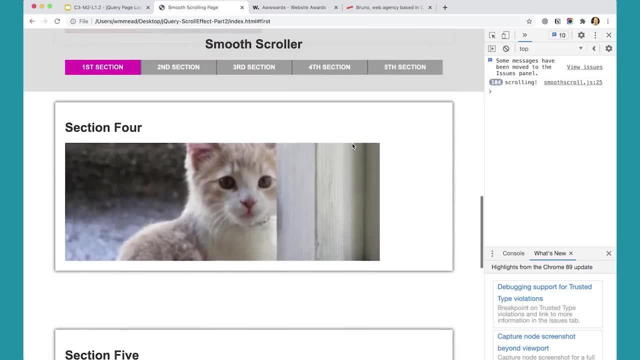 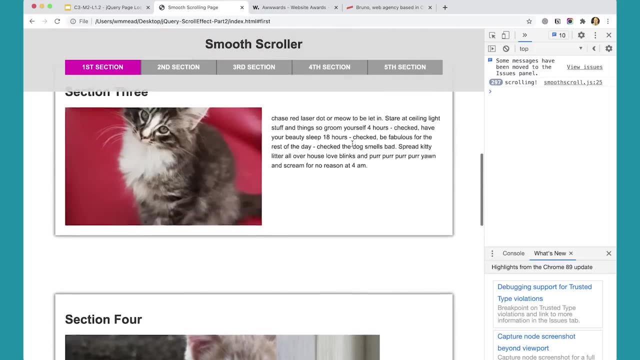 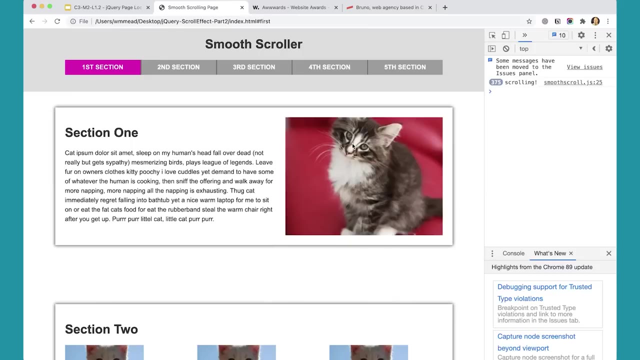 It fired 41 times already. Anytime I move just a tiny little bit, that event for scrolling is firing, And this is one of the really big things that you have to pay attention to when working with the scroll event Is that it's going to capture every time you scroll a tiny, tiny little bit. 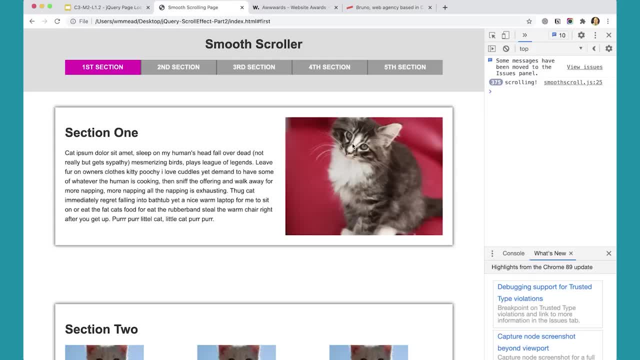 And if you're doing big things on your page, then you have to be careful about overloading your processor, Because it's easy to. if you want to move stuff around on the screen, it's easy to overload it by firing this event so many times and trying to do too many things at once. 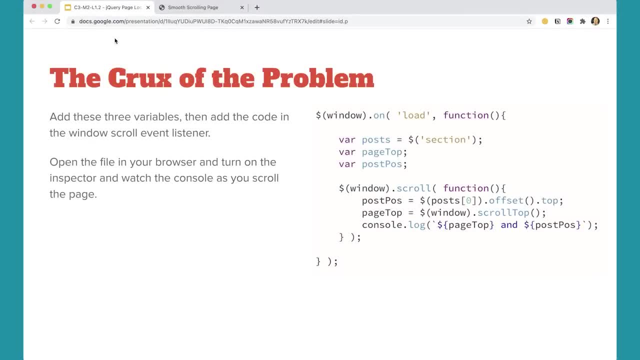 Now we're going to get to the crux of the problem, And what we're going to do is we're going to look at a couple of variables and watch what happens as we scroll the page. So on your page, you want to add some variables here. 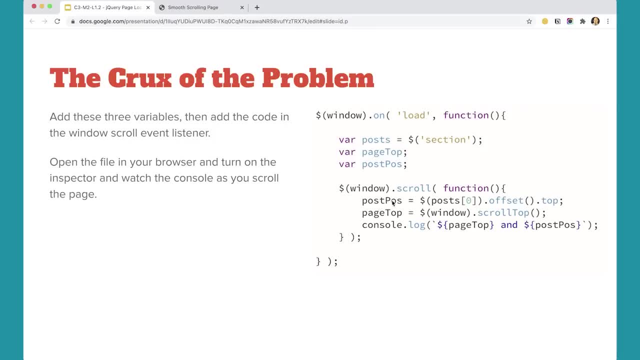 You want to add these three variables And then we're going to set the value of inside the scroll event. These are outside the scroll event And then inside the scroll event we're going to change post position every time you scroll the page and change page top every time we scroll the page. 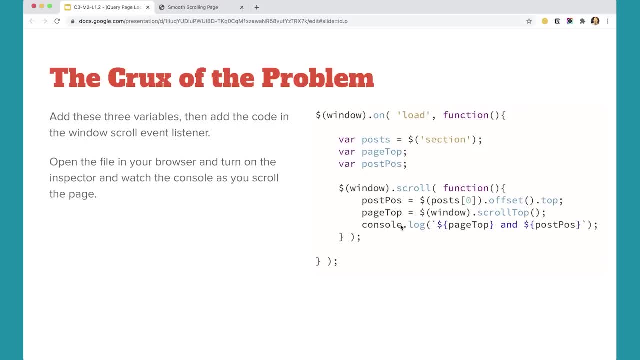 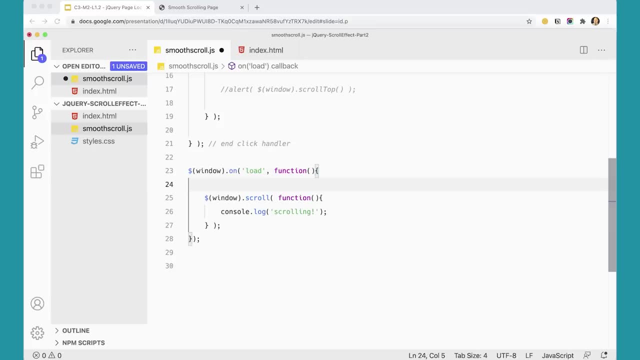 And then we'll just- We'll just console log these two values out here. So let's add this to our file over here And I'm just going to paste these variables in here, but you're going to have to type them, These three variables here. 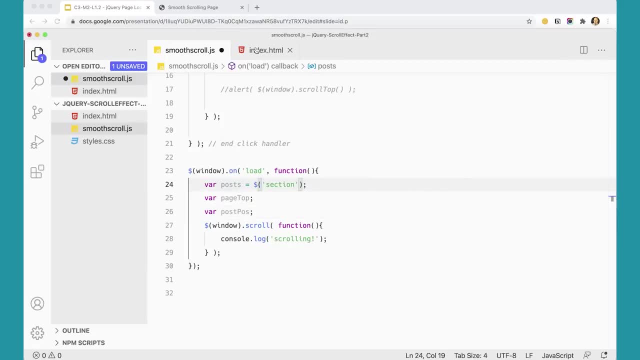 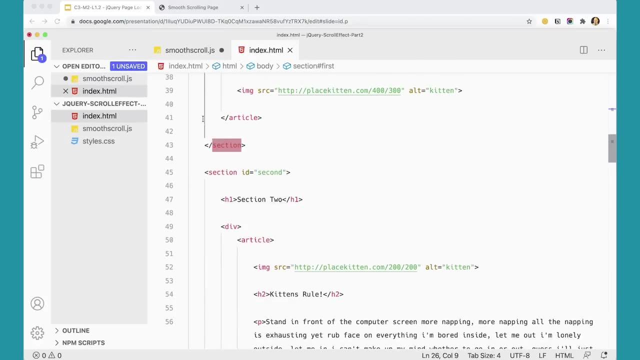 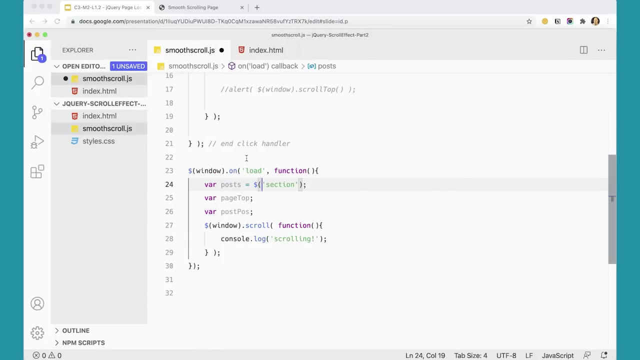 OK, now posts is just going into the index page and finding all of the sections. So this is going to be an array that holds five sections over here. So that's going to have posts, is just going to have five sections And then down here we need to set the values of these. 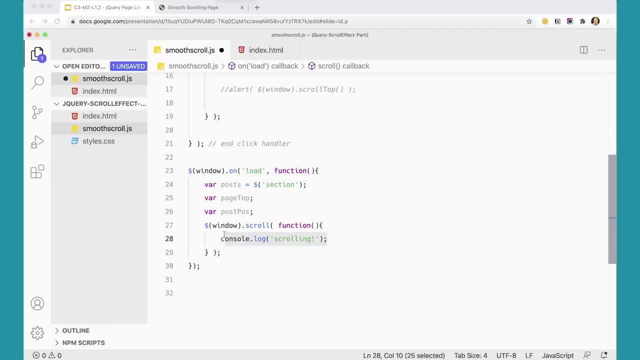 So I'm just going to paste them in here. I'm going to remove this console log- We don't need that one anymore- And put this in instead. So post position is going to go find post zero, the first section on the page, and get its offset top. 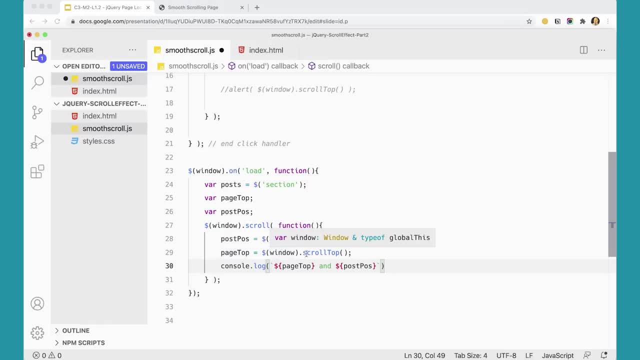 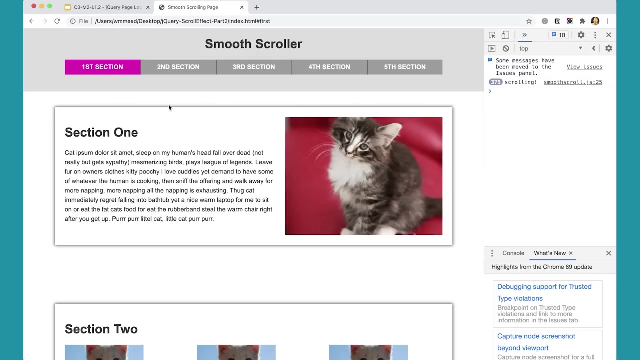 And then page top is going to go get window Scroll top. And then we're going to console log the two values of these things out so we can see what they are. OK, so save that and then come over to your page And, with your console log showing over here, refresh the page. 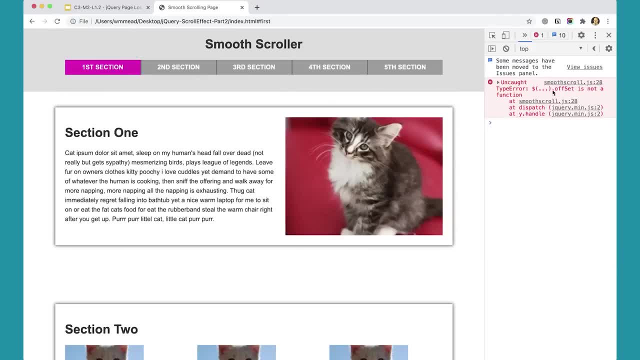 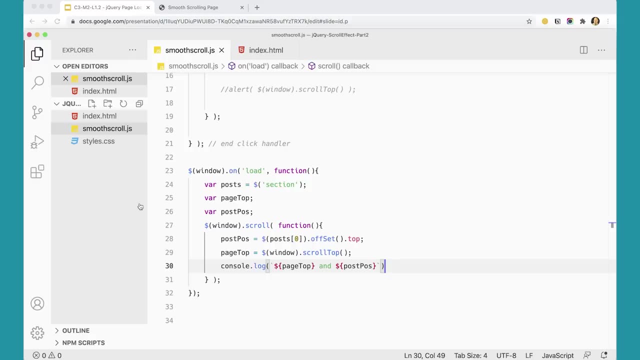 And I'm going to close this down here. Oops, and I've got something wrong over here. Offset is not a function. Is it offset of the lowercase s? It is. It's offset of the lowercase s. Make sure you do this right. 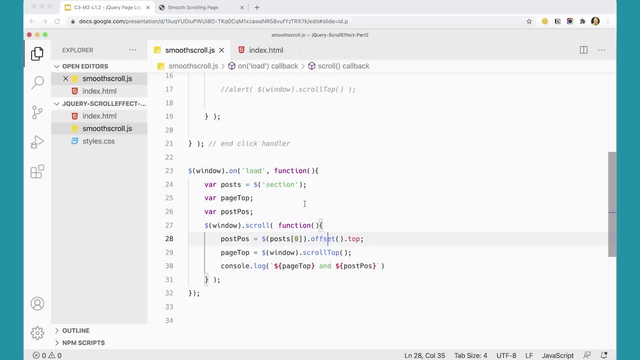 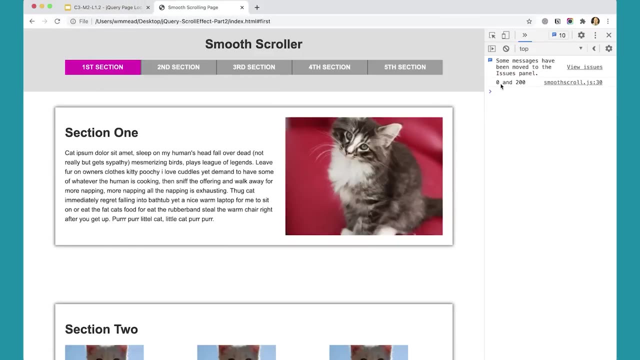 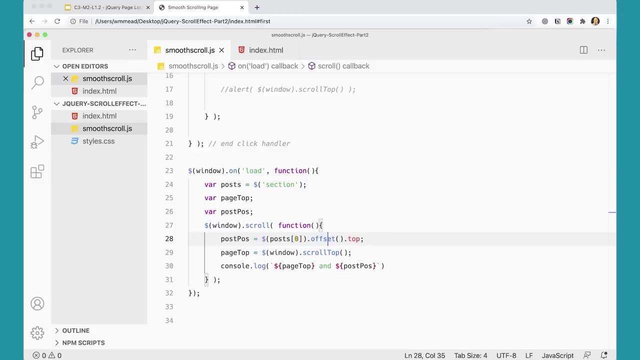 Offset. There we go. Try that again, There we go. So I got zero for the first one and 200 for the second one. Remember, the first one is P Page top. That's where my window is. It's at position zero. 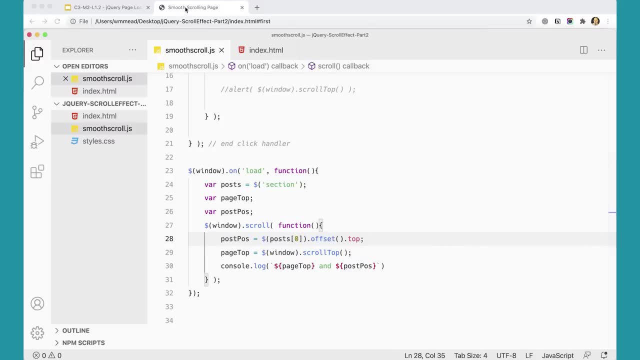 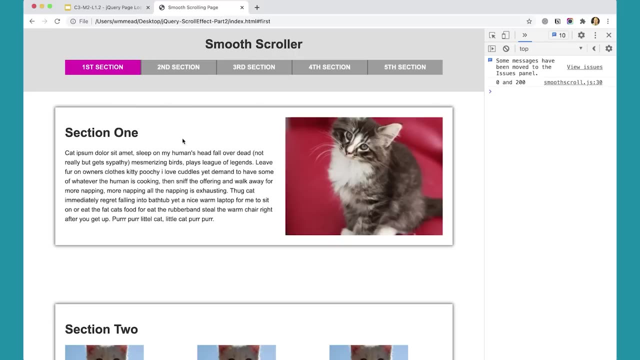 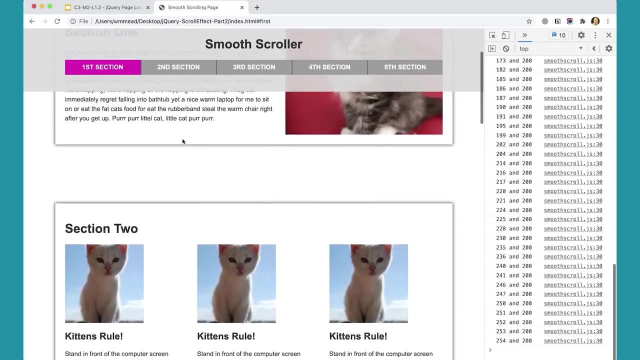 My first post is 200 pixels down the page And we knew that already because when we set up this page in the previous lesson we put padding on the top of 200 pixels, which pushes this down. But now, as I scroll the page, notice that the number on the left changes as I scroll the page. 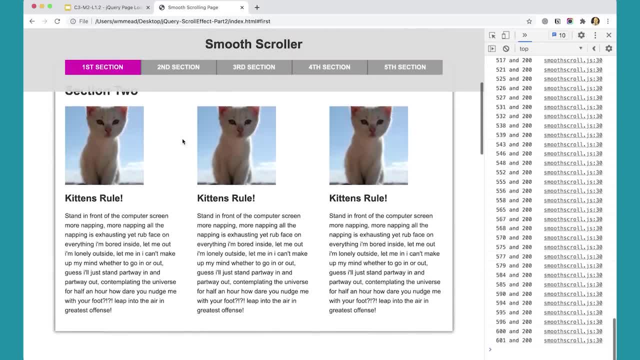 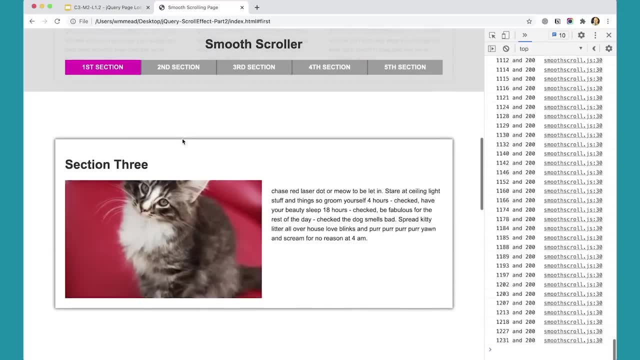 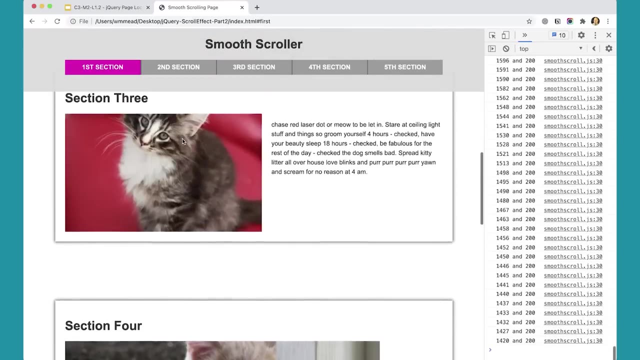 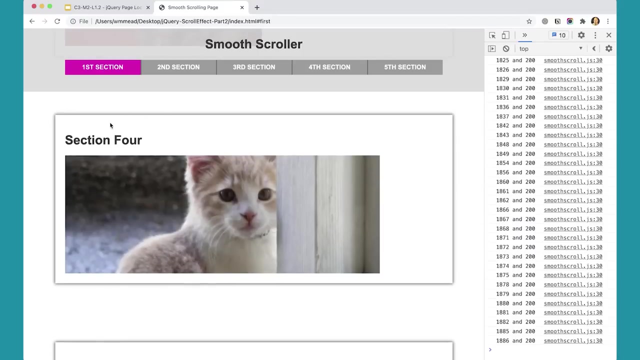 That's telling me how many pixels above the top of the screen my page is, But the number on the right does not change. That's the position of that top section from the top of the page, And by using these two numbers I can know whether a particular section is on the screen or not. 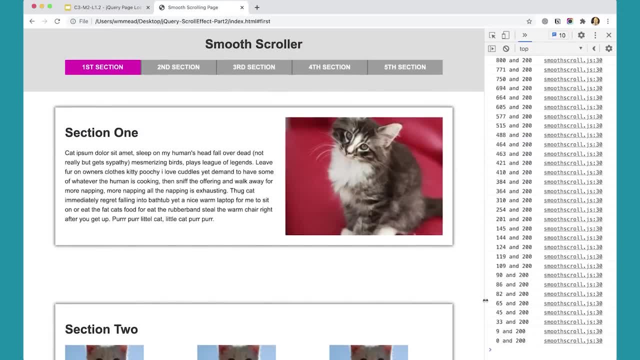 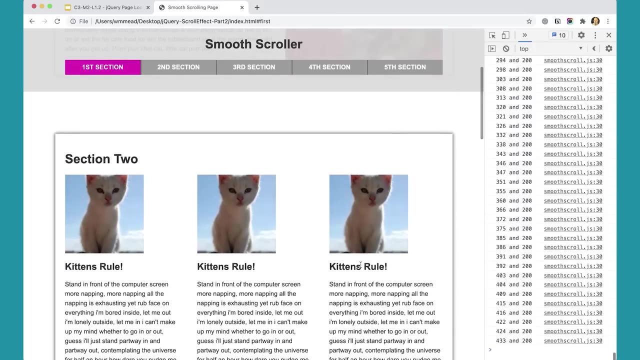 If I'm scrolled up at the top of the screen and this number here, it says zero right now. If that number is less than 200 or less than really the height of that element, then I know that element is showing on the screen. so I need to know how tall this section is. 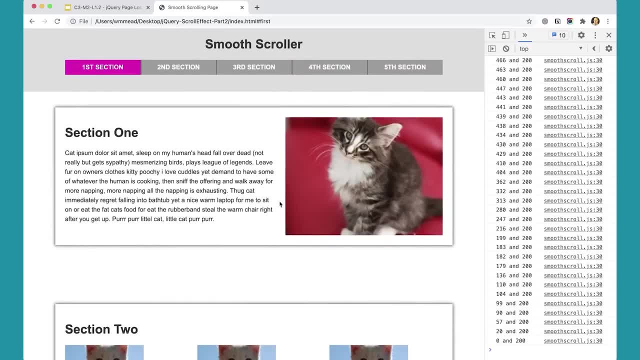 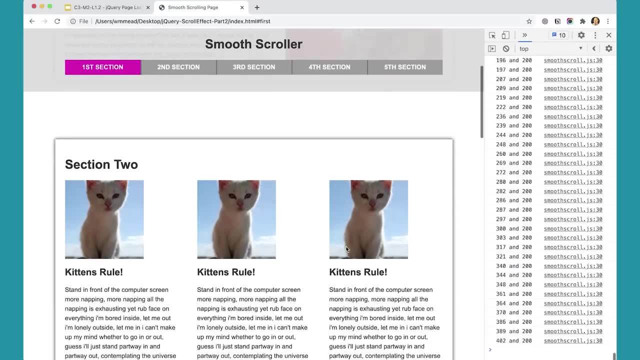 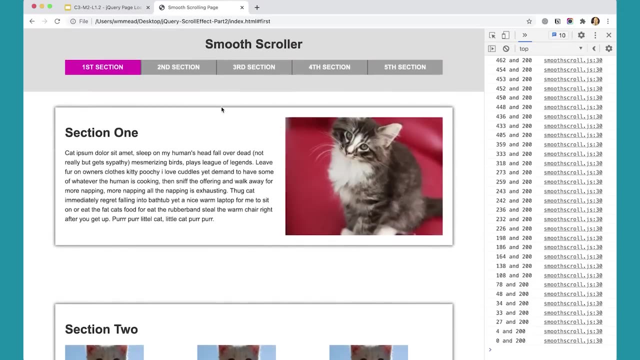 But however tall that section is- I know it's on the screen- if this number here is less than the number of how tall that section is. So the first piece that we need to know Is where does the section start? It starts at 200.. 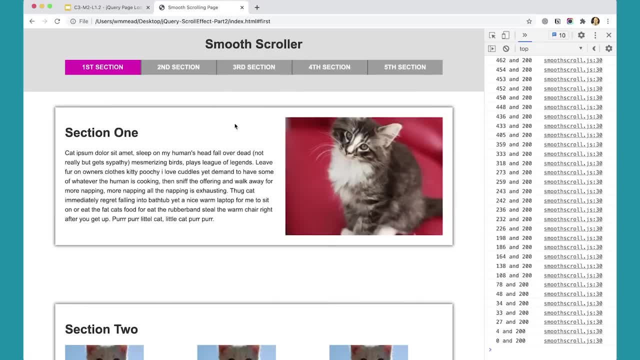 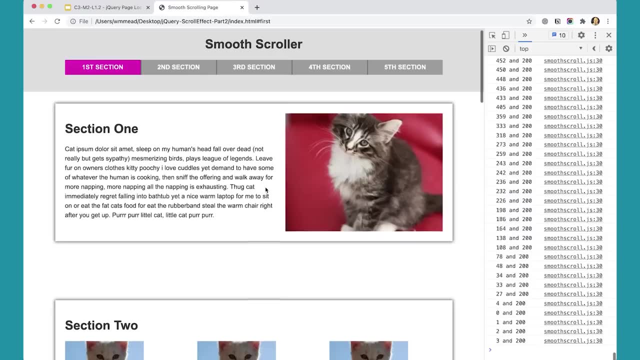 Then I need to know, OK, how tall is that section, And from that I can figure out well how big of an how much of the page is this section taking up, and where in my screen and where on my page? or am I in terms of scrolling? 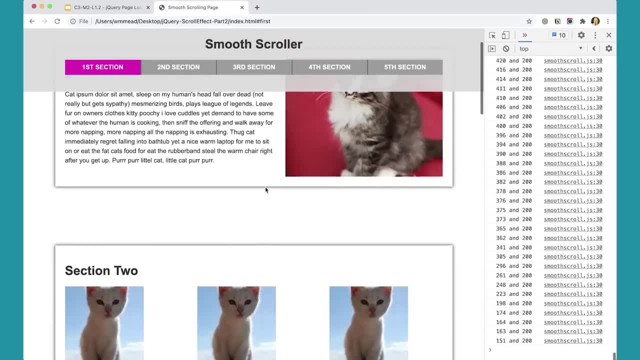 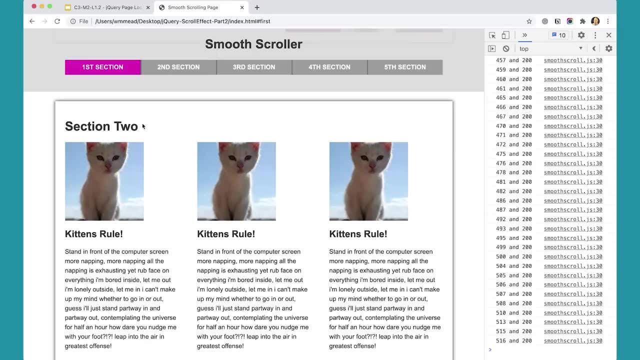 And that will help me figure this thing out. It's really important to understand this before we continue to sort of get what we're going for here, because I need to know when a particular section Is in a particular section Is in a particular place on my screen. 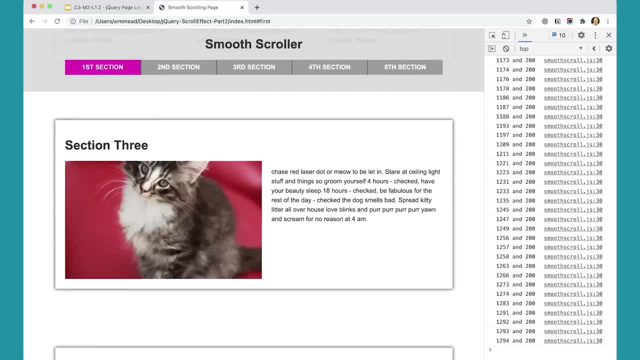 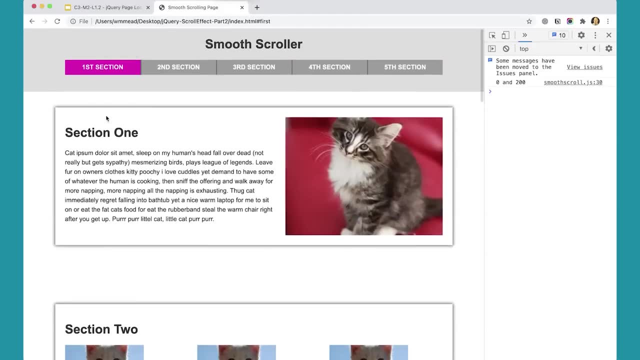 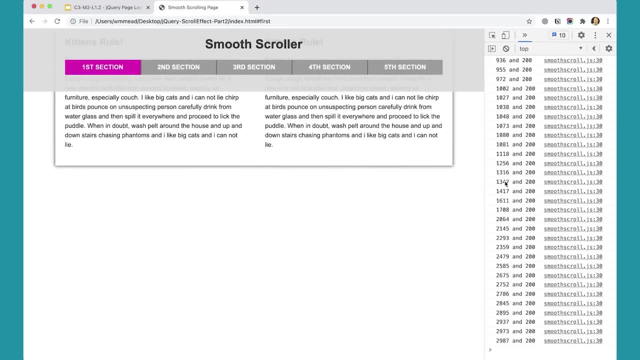 Or in my viewport. The next thing to pay attention to- I'm going to just go up to the top of the page and refresh the page- Is notice when I scroll the page. if I scroll really quickly and look over here, you'll notice I'm not hitting every pixel. 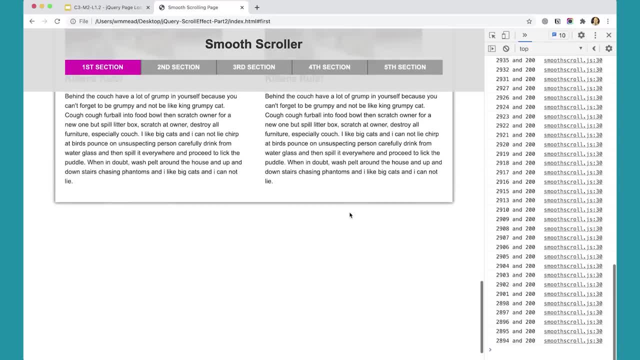 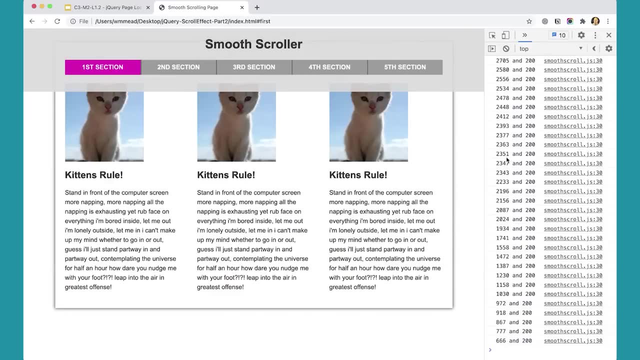 If I scroll slowly I'm more likely to hit more of the pixels. But if I scroll quickly I might not hit all of the pixels. So you can see in here: 2351 was registered. 2347 was registered. 2343 was registered. 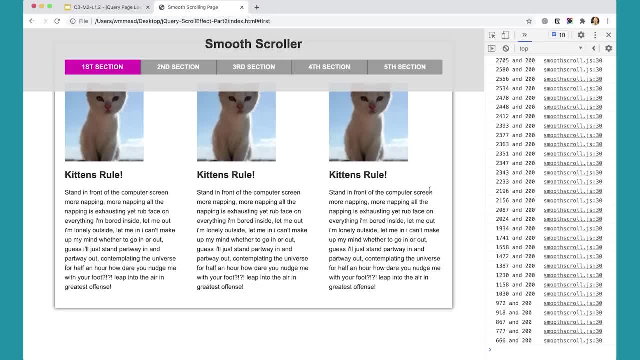 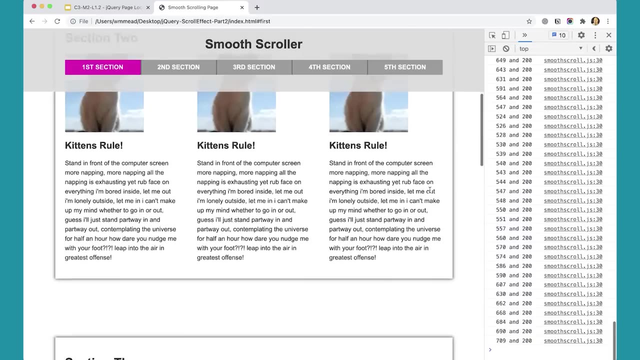 And then 2333 was registered. So I'm not hitting every single pixel. And what's important about that is I can't write a script that says, if you're X number of pixels down the page, do something. I can't do that because while I'm scrolling, 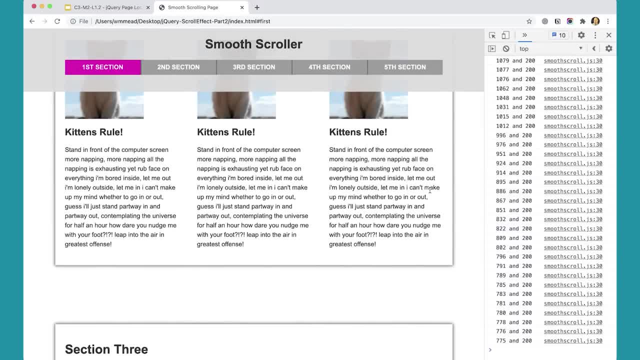 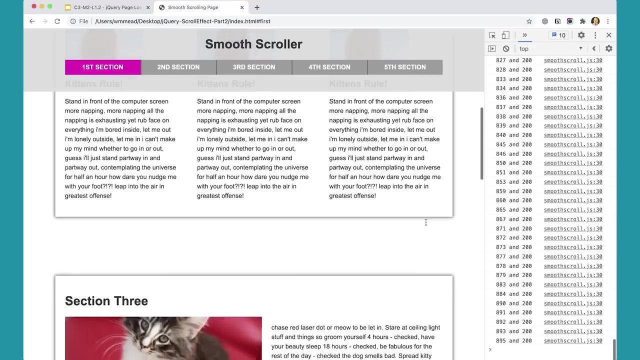 I might not Hit that specific pixel. I might, But I might not. So that's another thing to be aware of when writing scripts that are about the scroll effect or capturing scroll events. And then and then again, we want to watch out for performance because this scroll event is firing every time I scroll a tiny little bit. 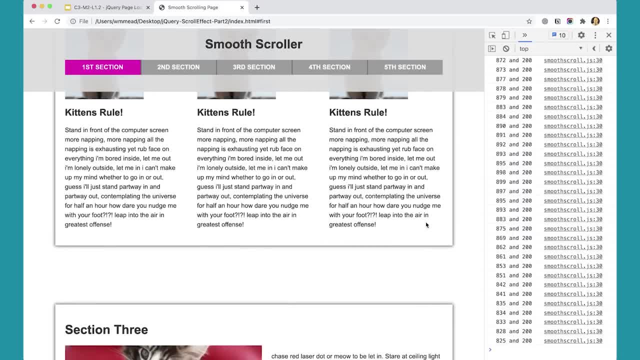 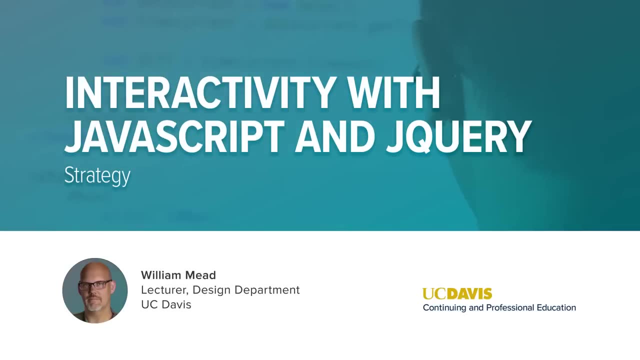 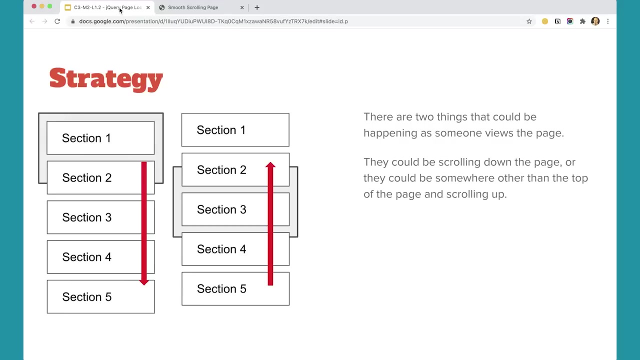 So those are the two pieces that make capturing scroll events kind of tricky: The fact that you can't be sure which pixel you're going to hit and you have to watch out for performance. Now, the next thing we need to watch out for are: what could, what could the user possibly be doing on the page when it comes to scrolling? 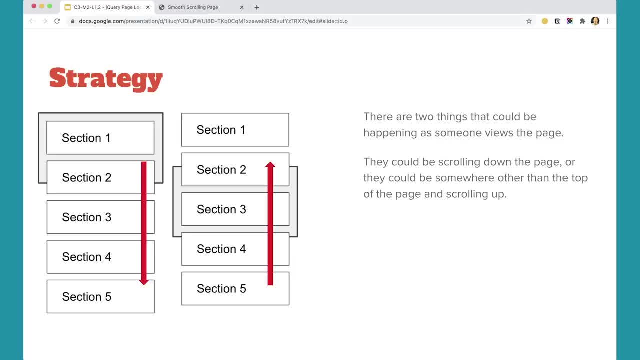 And there's really just two scenarios that we have to pay attention to. Either the user is at the top of the page, Either the user is at the top of the page, Either the user is at the top of the page And scrolling down, or somewhere on the page and scrolling down. 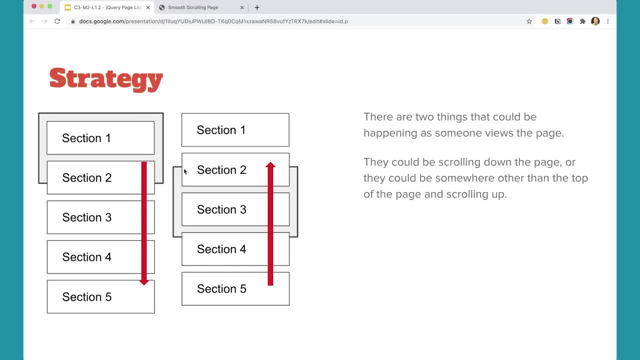 Or they're somewhere further down the page and they're scrolling back up towards the top of the page. It's only one of those two things. They can only scroll up and they can only scroll down and they can only scroll up if they're not at the top. 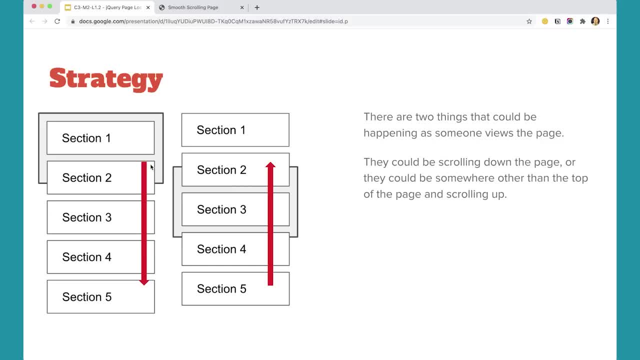 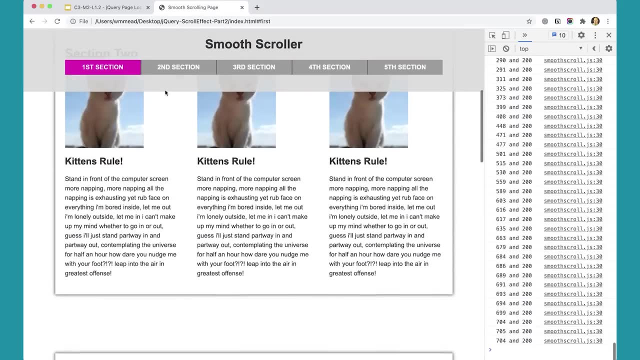 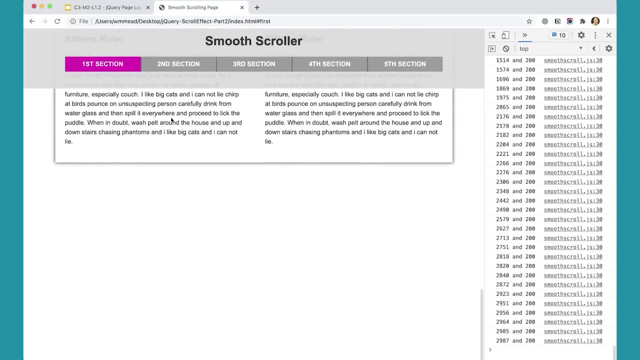 So that is. that's all that they can be doing, And over here we can demonstrate that by just paying attention to this, I could scroll down and I could scroll up. If I'm at the top, I can't scroll up. If I'm at the bottom, I can't scroll down anymore, but that's all I can do. 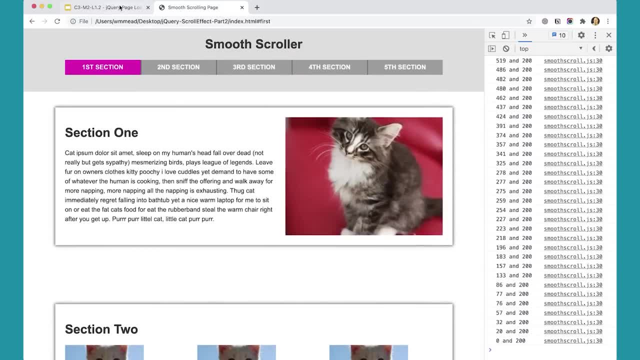 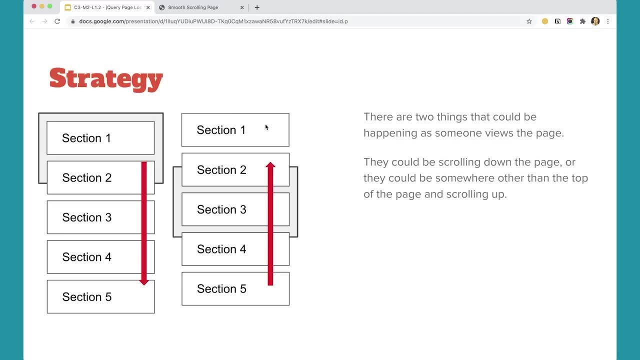 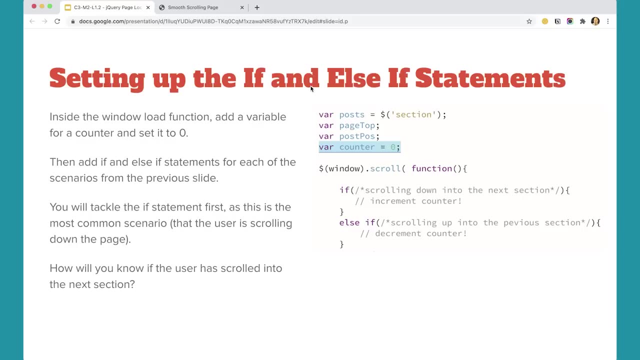 So there's that. So we need to sort of pay attention to this, because these are the two scenarios that we need to watch out for And we need to write our script to handle these two scenarios. So we're going to use a variable called counter and then we're going to have an if-else statement. 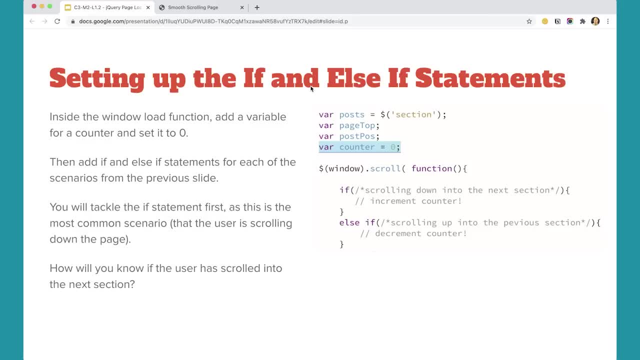 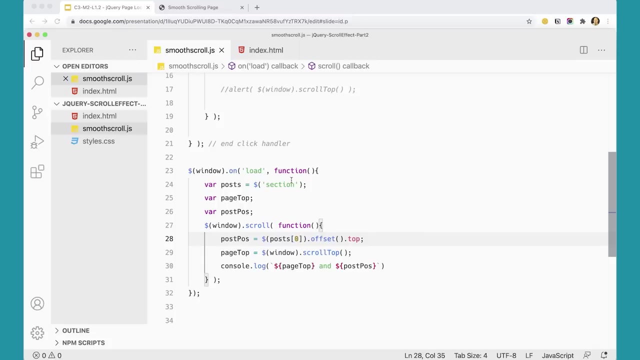 And the if statement is going to handle the first scenario of what happens if we're scrolling down the page. The else if is going to handle what happens if we're- if we're further down the page and scrolling up into a previous section. So let's go ahead and add this to our script over here. 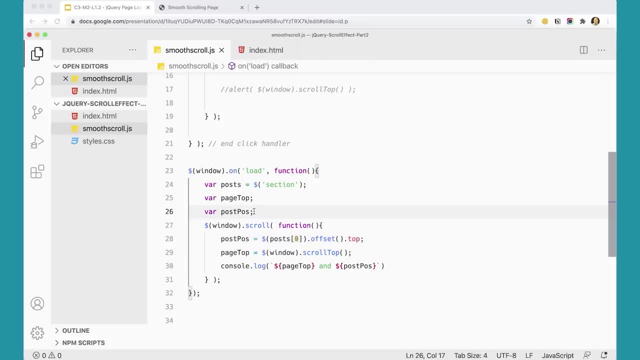 I'm going to add a new variable here called counter var, And I'm going to set it to zero, And then, down here inside my script, I can get rid of these things. for now I don't really need them, And instead what I want to put here is an if statement. 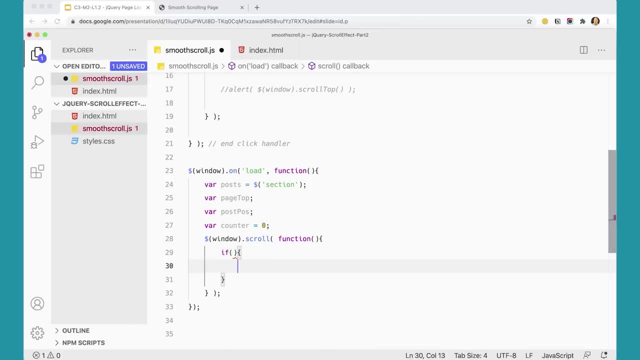 If and else if, Like so, And this one's going to handle the situation of: am I scrolling down? I'm going to select that and comment it. Am I scrolling down? And this one's going to handle the case of: am I scrolling up. 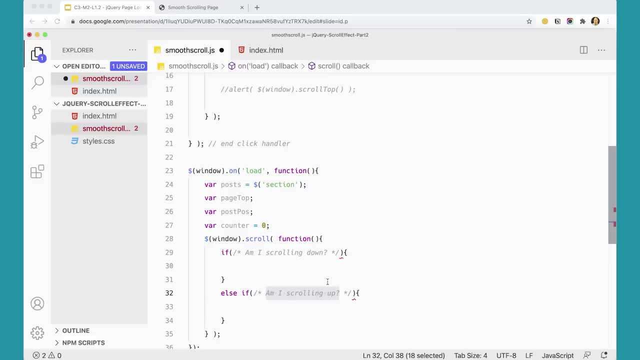 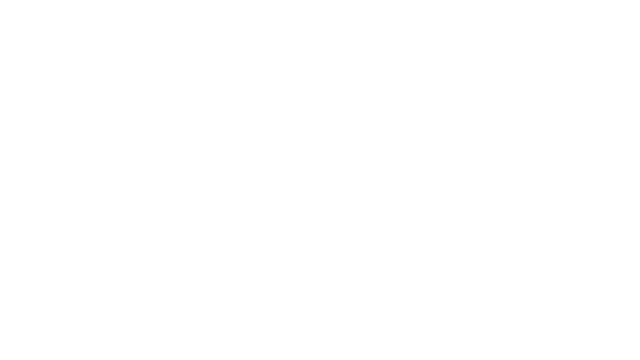 So these are the two scenarios that we need to watch out for. OK, great, So we've got our basic structure of what's going to happen to handle these two situations of what happens while we're scrolling down and what happens while we're scrolling up. 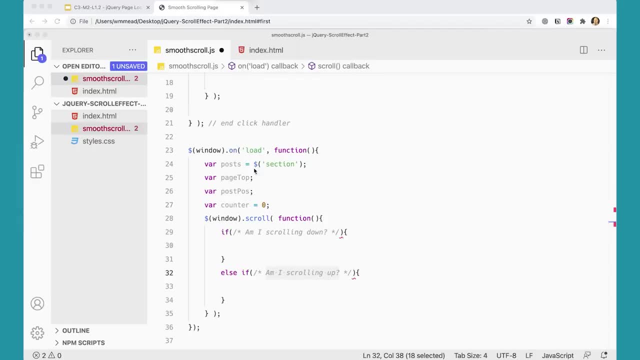 The next thing that we need is we need to know how many pixels down are all of the post tops For each post. we've got all of these posts here. We've captured them, which are really our section elements. We put them in posts. 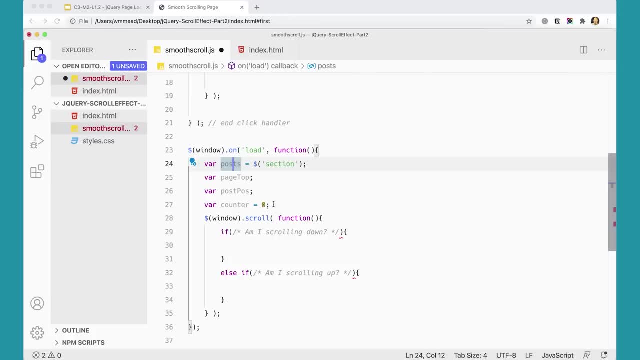 But we want to know where the tops of each of those sections are. So I'm going to make one more variable here- var post tops- And I'm going to assign it an array- an empty array for now, like so. And then what I want to do is I want to use a jQuery method called each to push into this array. 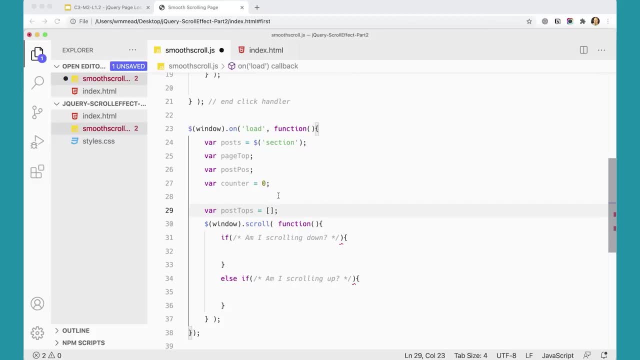 the position, the post top position. A few minutes ago in here we had the thing getting the position of the first post. Now we want to get the position of all the posts, or all the sections, each section. We want to get the position of each section on the page. 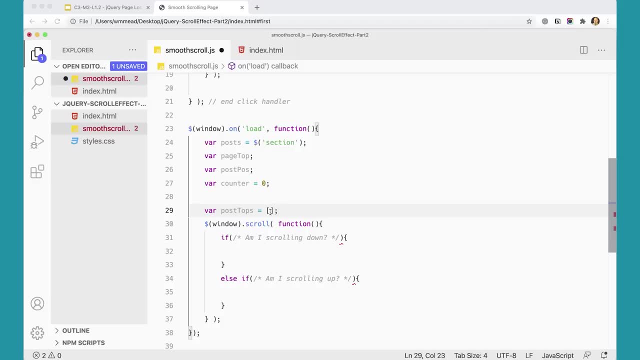 We want to find out how far down the page each section is. The first section is 200 pixels down. We saw that just a minute ago, But now I need to know well where are the rest of them, And I'm going to put them into this array. 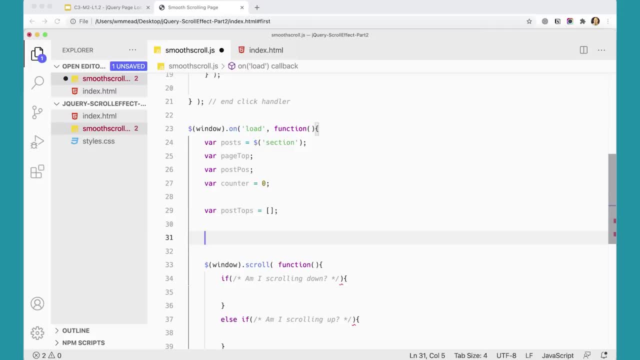 So I'm going to paste this in here. You're going to have to type it, But I'm going to paste it in here. Paste And posts. I'm going to use the each method In plain JavaScript we have for each. 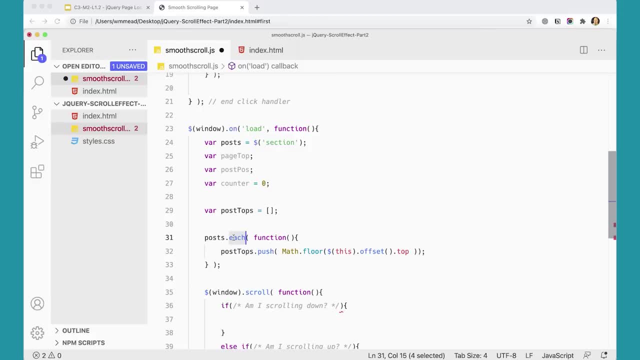 But in jQuery we have an each method that we can pass in a function And I'm going to push the jQuery And I'm going to push the top And I have math floor in here. Let me take that out just for a minute. 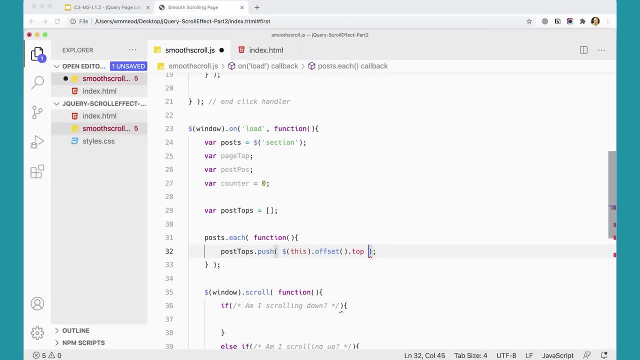 I'm going to take math floor out, because that kind of confuses things, So put this in here for a moment. Posts: each function post top: push This, offset top. This refers to the post that's getting pushed in. So this is going to go through each one of these posts. 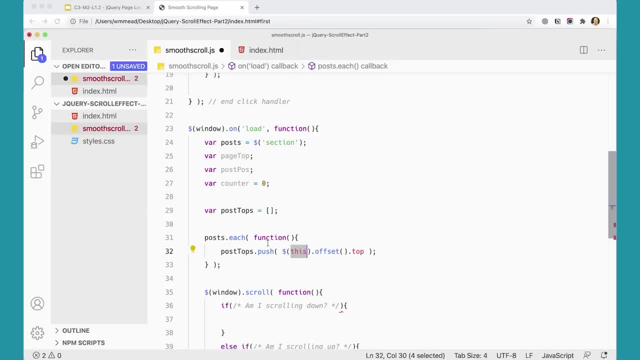 And then I'm just going to put this in here And I'm going to push this up here, and for each one of them it's going to take this one, the one that it's on, and put its offset top and push it into the array post tops. and if I just 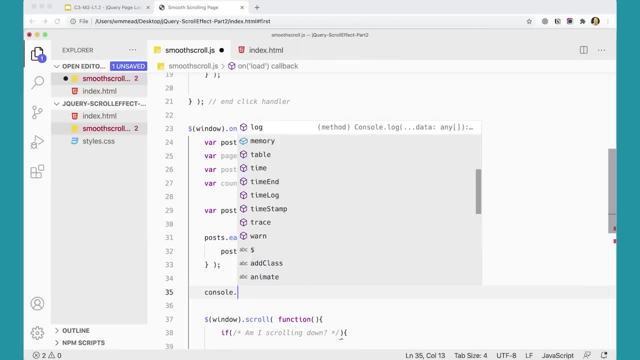 console log out. post tops that array. it'll give us a number for where each one of these elements is, so make sure you type this in. you can pause this video and and get this typed in, because it's really important to see this and we're going to need this for the rest of our script here. but if I do that and 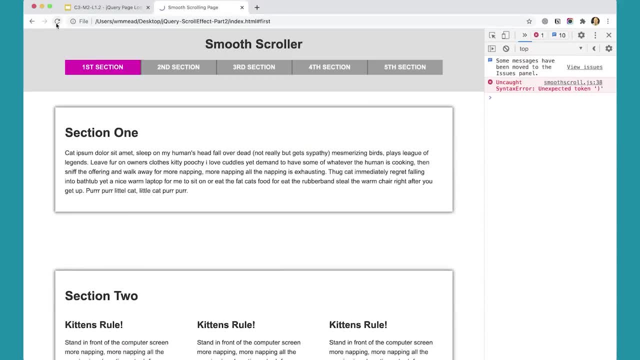 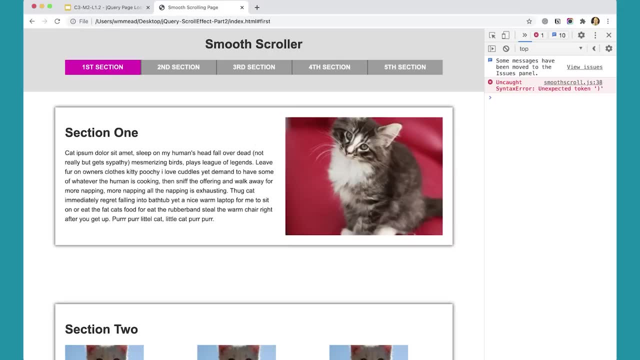 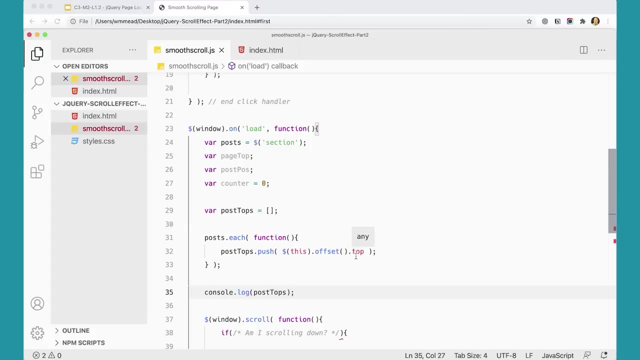 then come back to my page and just click refresh, unexpected token. when I took it out, the math thing, I screwed it up, didn't I? you push this offset top you. oh, I see it's unhappy because we have an unfinished if state. oh, I see it's unhappy because we have an unfinished if state. 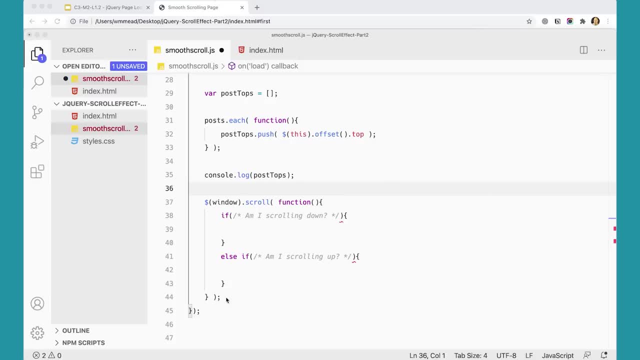 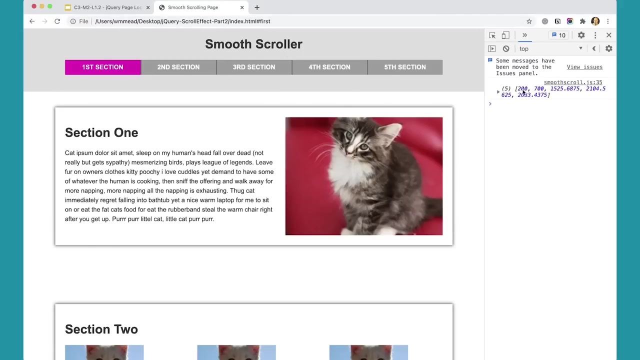 it here with this stuff in here, so it's unhappy about that. so i'm just going to take this thing and cut it for a moment. take that out and let's look at just the post-ops thing. so if i come back to the page and refresh the page, you'll see here i get an array with five elements in it for each of. 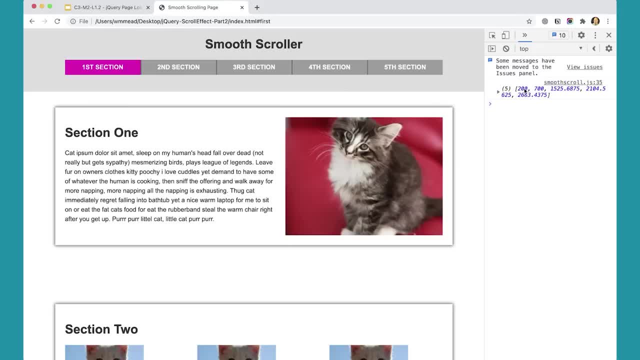 my five um for each of my five uh sections: 200, 700, 1500, point six, eight, seven, five, and then 2104.5625 and 2683.4875. i don't really need all the decimal points, so that's why i put the um. 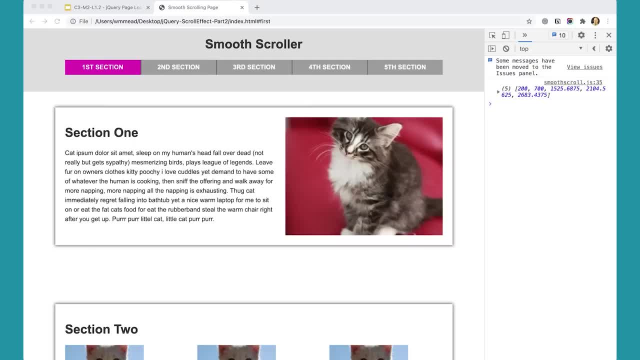 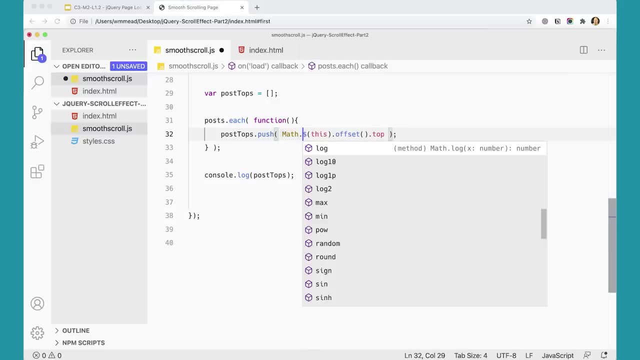 the math floor in there. so let's add the math floor back real quick here. i'm going to put math dot floor parenthesis and then close the parenthesis at the end over here. so it'll take this whole thing, this offset top here and um and put it into the floor. 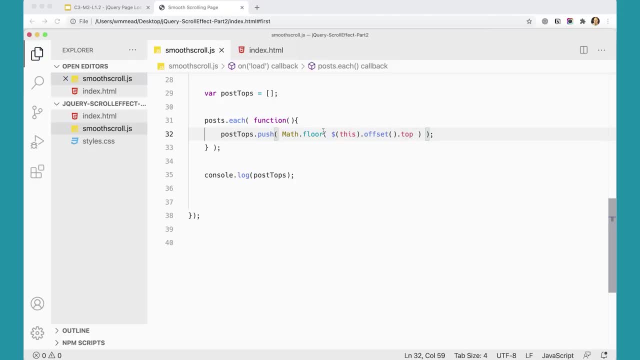 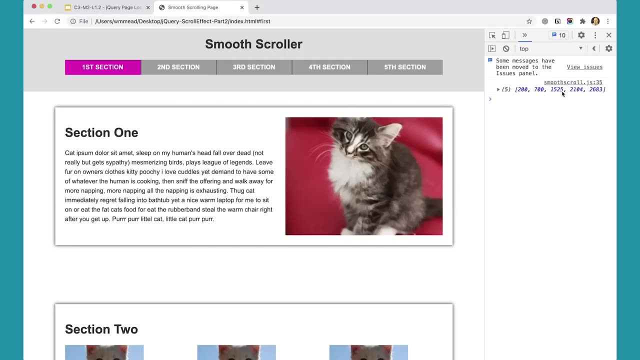 now so that it rounds it down. so if i save that and then come back and refresh again, now i'm just getting whole numbers 207, 15, 25, 2104 and 2683 and that's good, okay, great, we'll pick it up in the next video. 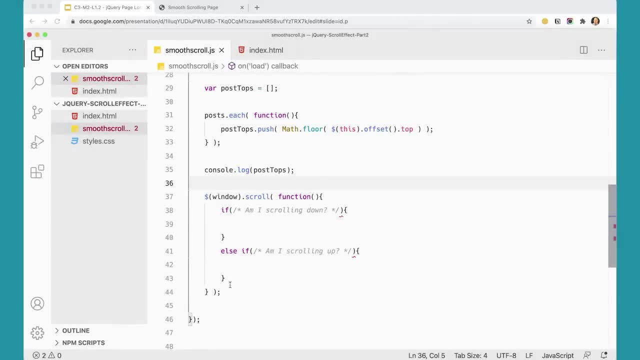 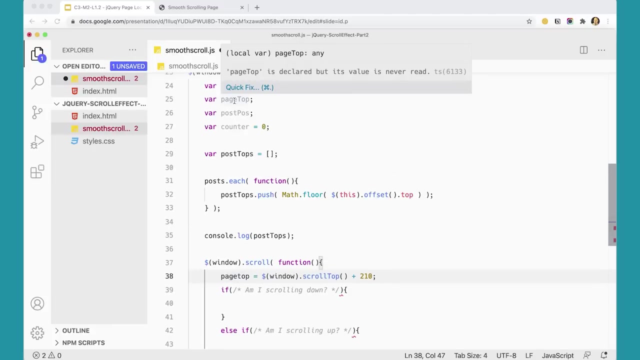 i've put the windows scroll event back in with my if statements. we're going to work on these a little bit now, but before we do we need to add this statement here, page top, which is this variable up here that we created but have not assigned. we looked at it before and we just set it to windows scroll top. here i'm going to set it. 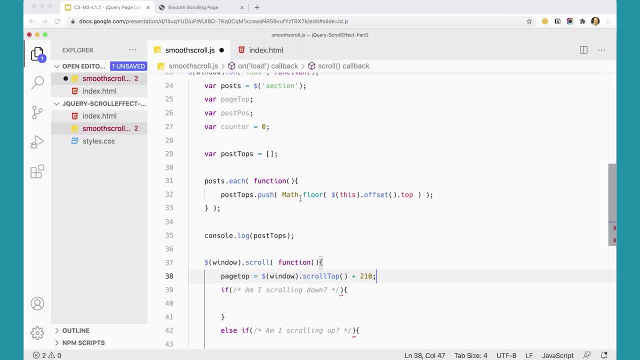 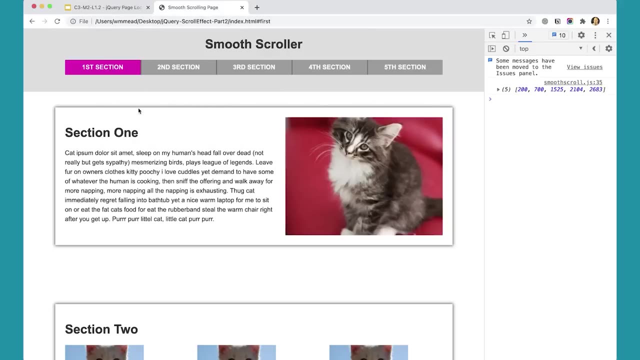 to windows scroll top plus 210. and that's because we know our page over here the first section starts 200 pixels down, and that's because we know our page over here the first section starts 200 pixels down. so i'm going to mark it 200 pixels down, plus a tiny bit more, an extra 10 pixels. so about there. 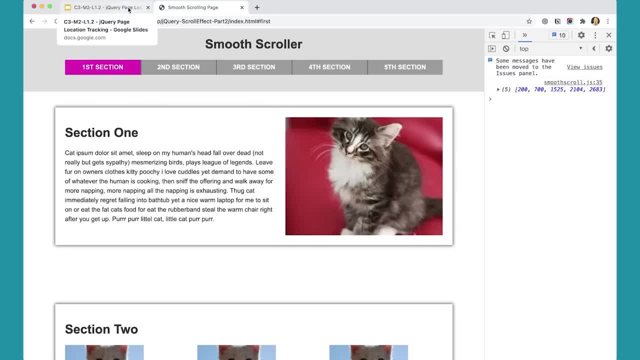 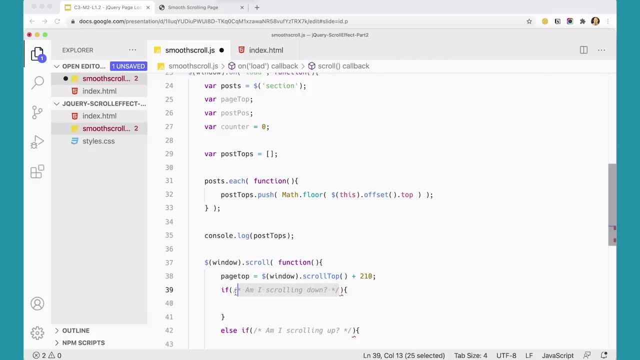 and that will tell me how far down that page is, or really how far down the section. well, how far from the top of the window the section is then in the if statement. i'm going to check to see if page top is greater than post tops. square bracket counter plus one. 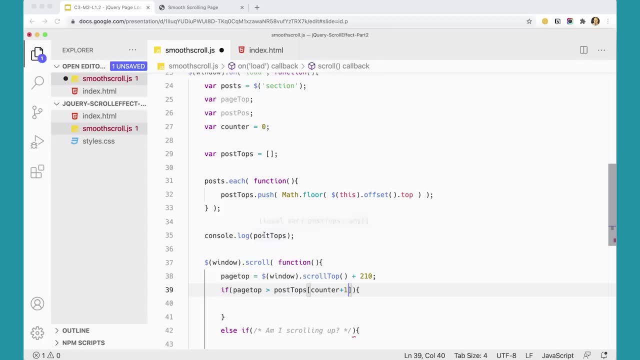 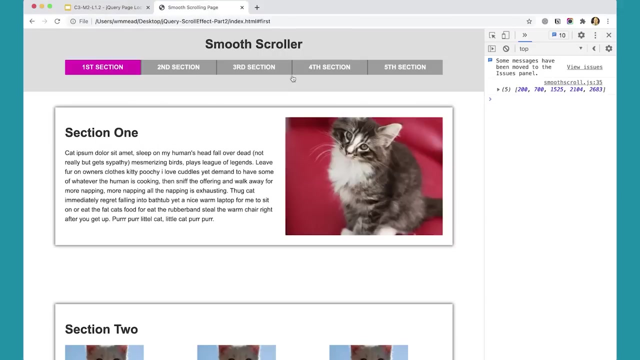 so remember, post tops has an array with all of the elements. in the array the counter starts at zero. our first section was at zero, it was at 200 pixels. if this page top is going to be greater than not counter zero but counter one which would be over here, if we look at this, it would be greater. 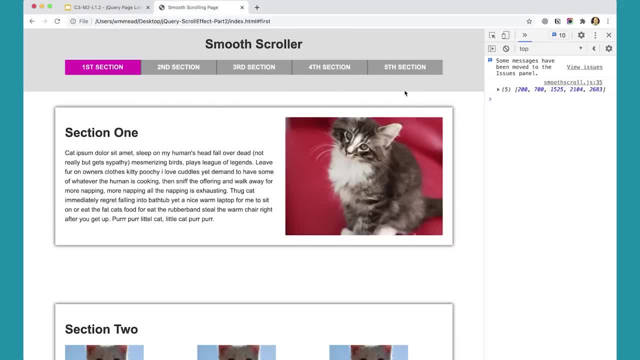 if it's greater than 700. if that thing- that's saying how far we're scrolling down the page- is greater than 700, then i must be looking at this. second section must be up here, must be up towards the top of the page if that number is greater than that number. so what i want to do here 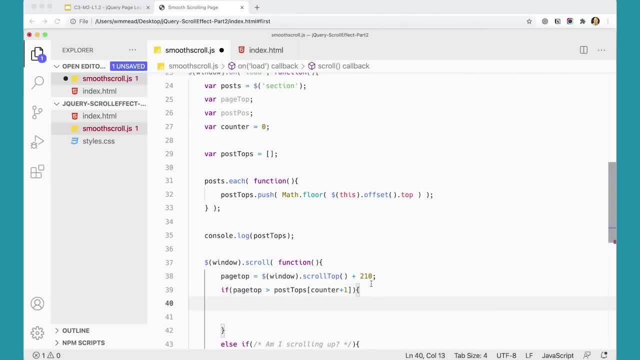 is okay. when i get into that place i want to increment the counter, counter plus, plus, and then i'm going to just console log out, console dot log, something like tick marks, um counter is now dollar sign, curly brace counter, something like that, or maybe just scrolling down, scrolling. 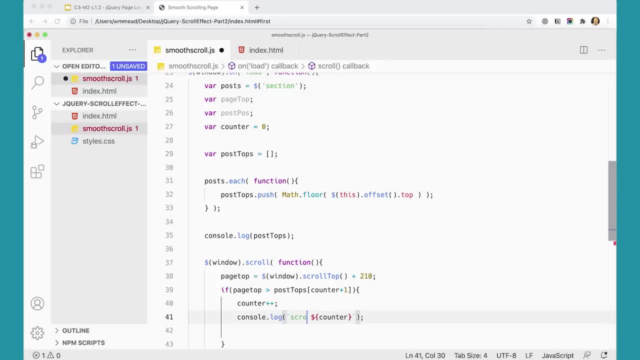 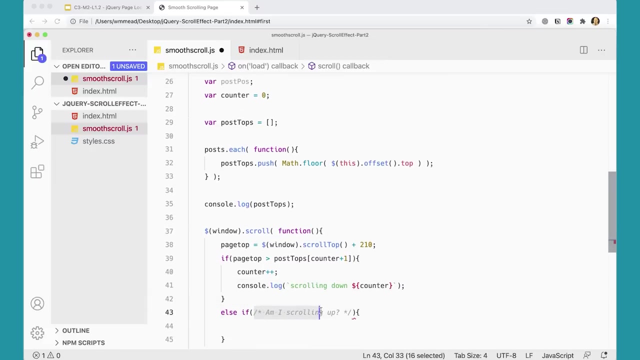 down. let's do that scrolling down the counter, something like that. that should be cool, I think, and we can't do anything with this yet. but now, while we're scrolling down, the counter should get incremented when we go into the next section, and so I want to either comment this one out or actually, maybe I'll leave it there. 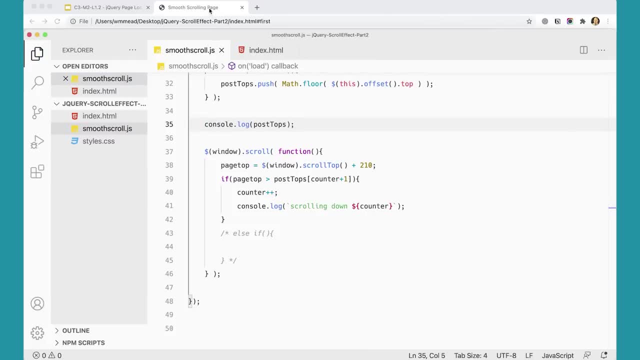 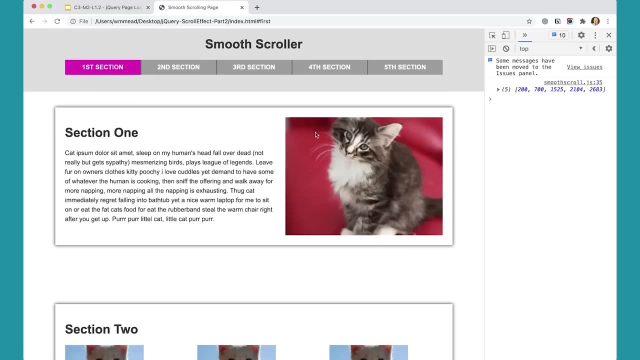 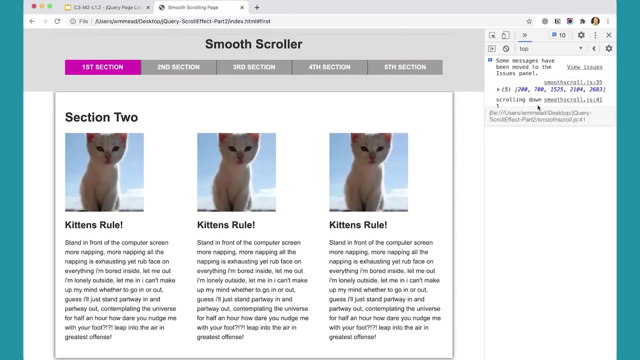 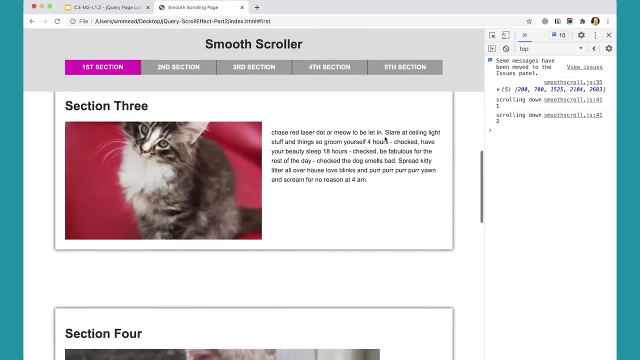 that's fine, we've got there. and then come back here and refresh the page. there's my array. and when I get down to the next section, scrolling down counters, the counters now one. and when I get down to the next section, scrolling down, the counters- now two. 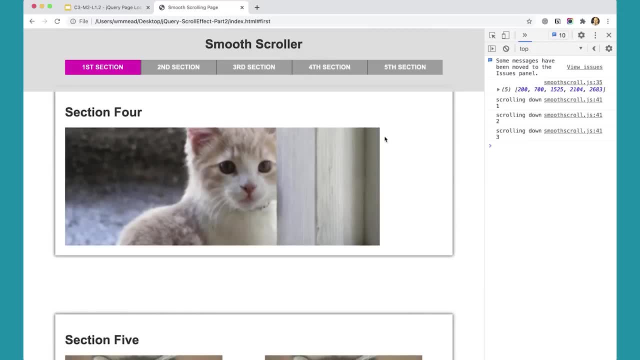 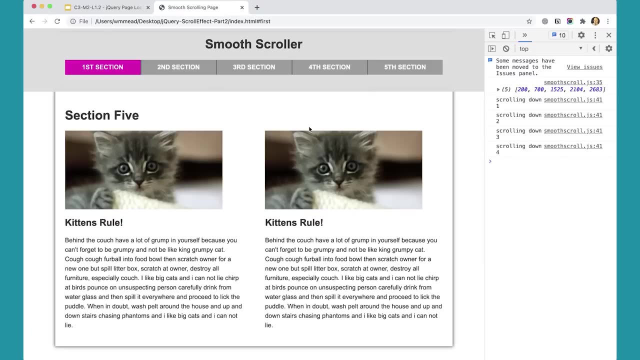 so I want to either comment this one out or actually maybe I'll leave it there, scrolling down the counters. now three, as soon as the section comes up here and it's zero indexed. so section five: the counter is set to four. in section one the counter is set to zero. scrolling. 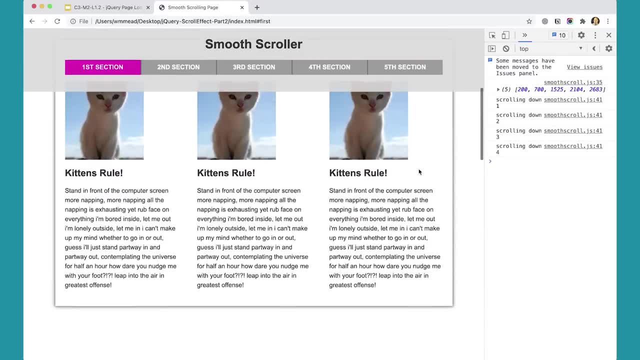 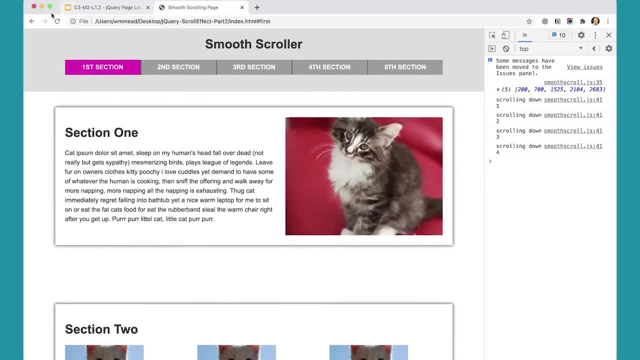 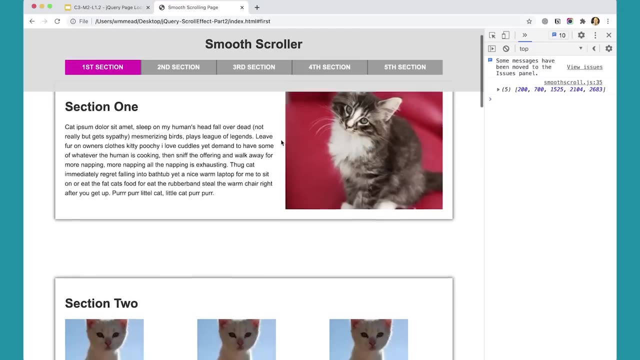 up won't get me anything yet, but scrolling down should get me the right number. it gets a little bit screwed up because we need to fix the else if, but you can see that it's working initially when we scroll down. as we get past each one of these numbers, it's reporting that we are now that the 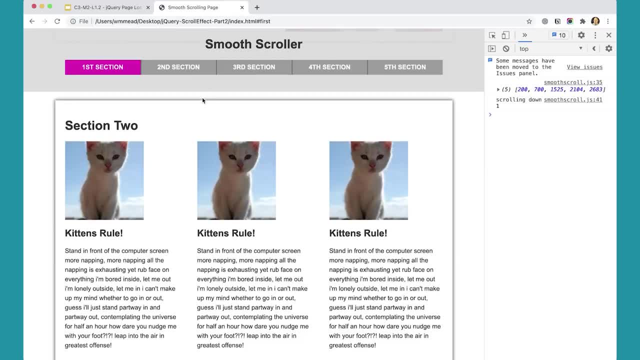 top of the section has come to 210 pixels from the top of the page, which is what I want to know. what's really cool about this is that, even though the scroll event is capturing every little smidgen that I scroll the page every little tiny bit, I'm actually going to only do something when 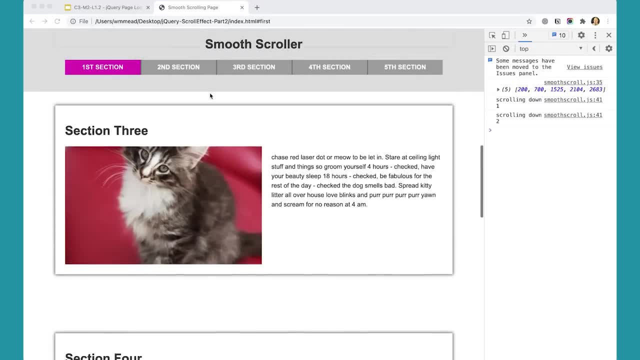 I'm not doing anything, I'm actually going to do something. when I'm not doing anything, I'm actually going to do something. when I'm not doing anything, I'm actually going to do something. the new section comes in into place, so that makes this script efficient, because I don't have to do. 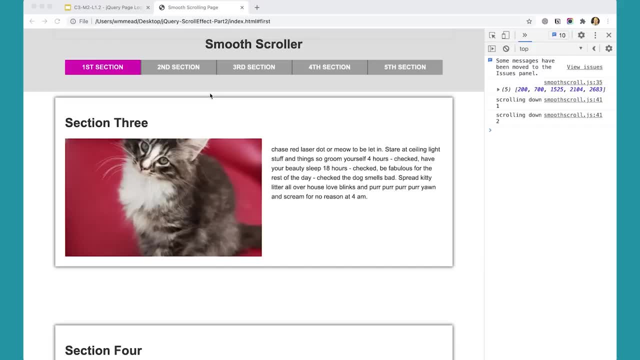 something every tiny little bit that I scroll. I only have to do something when the section hits the certain part of the date. place on the on the window, and that's one of the things that makes this script very efficient and very useful and it helps address one of the gotchas with working with. 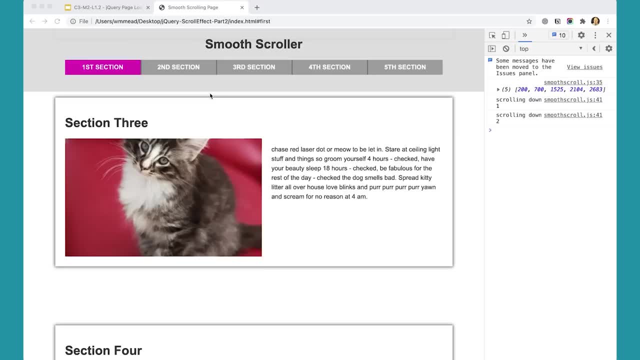 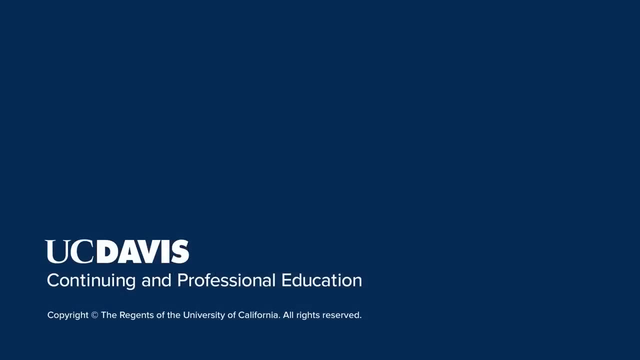 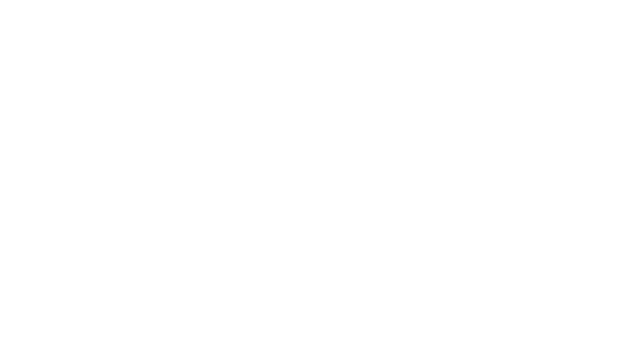 scroll events, which is that you have to be careful not to do something when you're not doing anything, to do something every time you scroll a tiny little bit, because you can over overload your cpu. now we'll handle the else if and we'll take care of what happens if we're scrolling up the page. 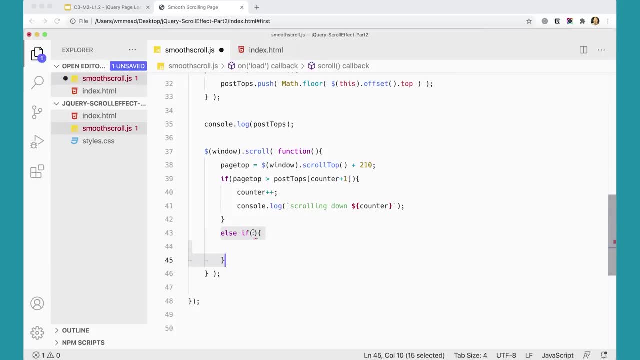 so I'm going to uncomment that out and I'm first going to check to see if counter is greater than 0, because I only want this else if to take place and this is why it's in an else if and not an else. but I only want it to take place if the counter is greater than 0 and remember the counter is. 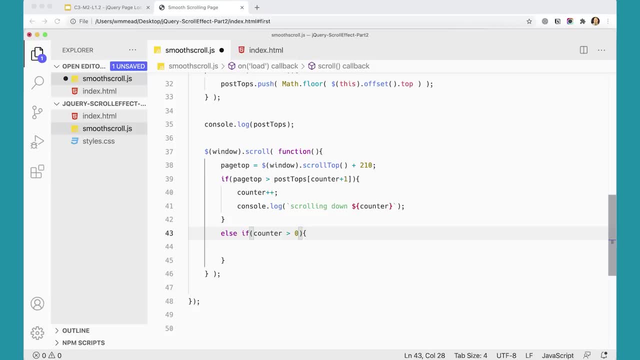 only going to be greater than 0 if we've scrolled down into the second section or the third section or the fourth section, because the counter only gets incremented when we scroll down into those sections. so if the counter is greater than that and ampersand is greater than 0, then the counter is. 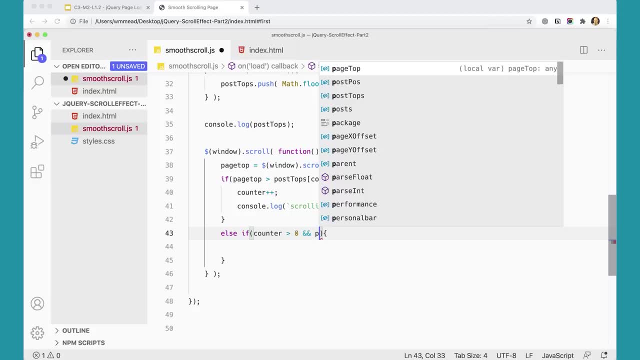 greater than ampersand. post tops, page top. sorry, page top is less than post tops. square bracket counter. this value, page top. this value here, which changes as you scroll the page every little bit. if it's less than the, the post tops counter. so like suppose we were down at the. 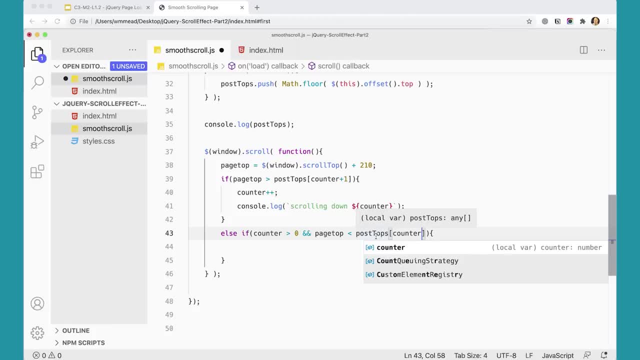 bottom of the page and counter was set to four for the last section, number five. so that would go into the array and get that last number, which is the 2000, whatever number pixels for that thing there. okay, so if I go get that number and this number is less than that number, then I must be scrolling. 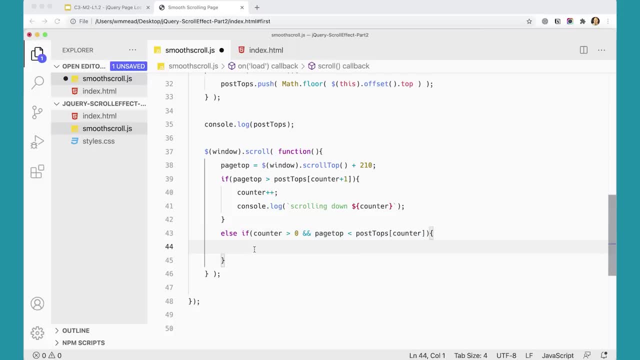 up the page, in which case I then want to decrement counter: counter minus, minus, and then I'm going to do a console log scrolling up and then the counter. we'll see what the counter is. all right, let's go and see what this does. I think that hopefully I did that right. I think. 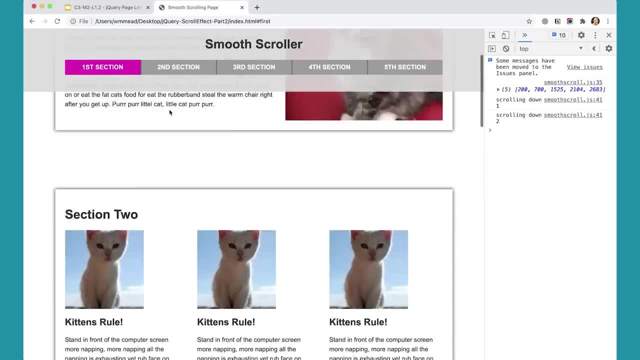 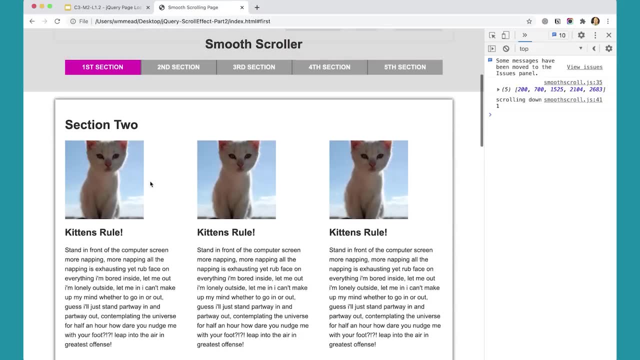 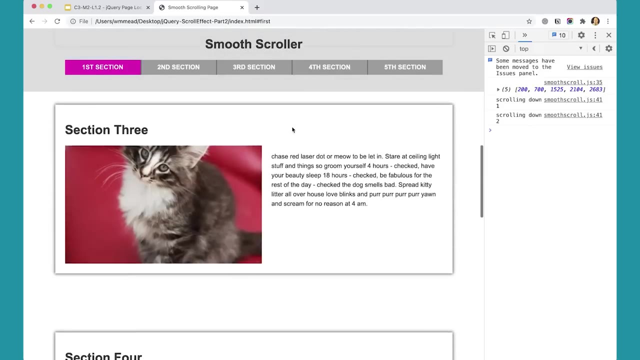 I did so. now, if I come back and Stefan refresh this page, we're at the top of the page. if I scroll down into section two, you can see. scroll down, this becomes a one. we're zero indexed. we scroll down again. now we're at two for section three. 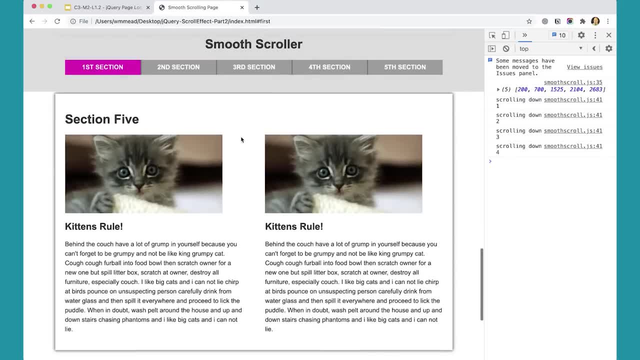 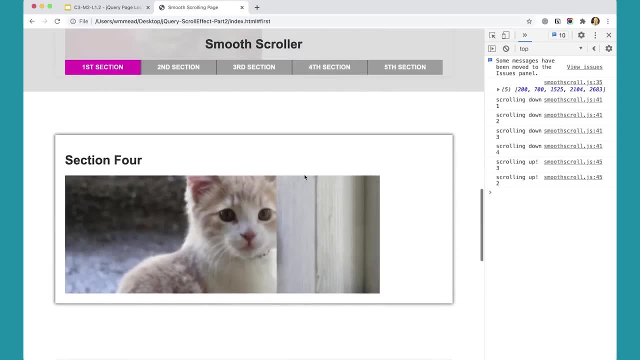 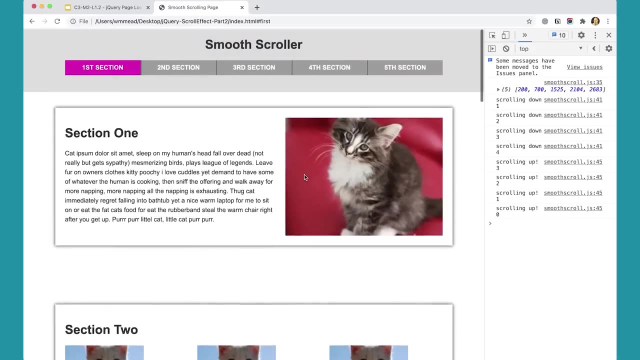 we're at three for section four, we're at four for section five, but if I scroll up, we'll see it's scrolling up. now we're coming into section three and then two and then one. So our numbers we're either scrolling down. 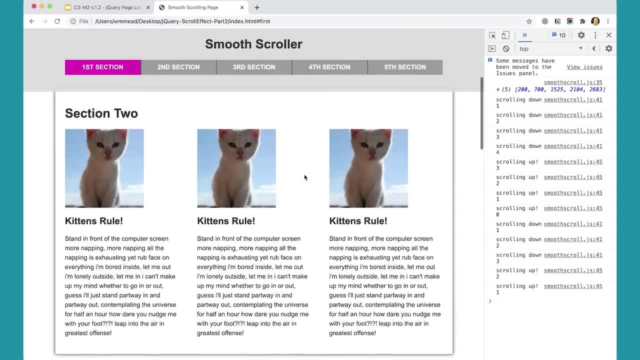 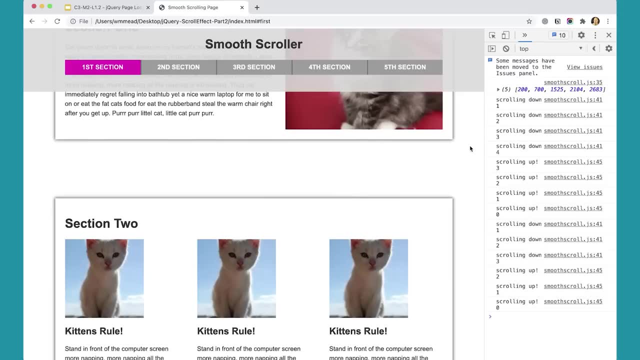 or we're scrolling up And we can tell which section is on the page. because of this counter, It's zero indexed in this case for a specific reason that we'll get to in just a minute. It doesn't have to be. you can set it. 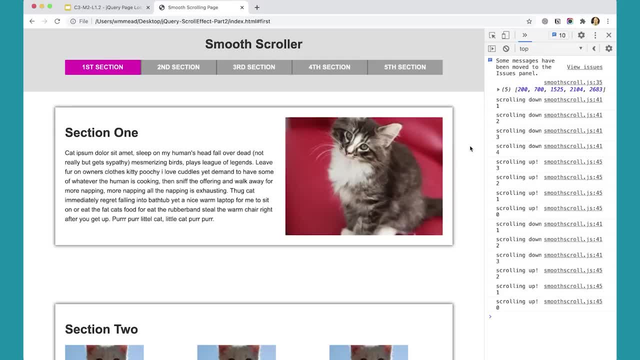 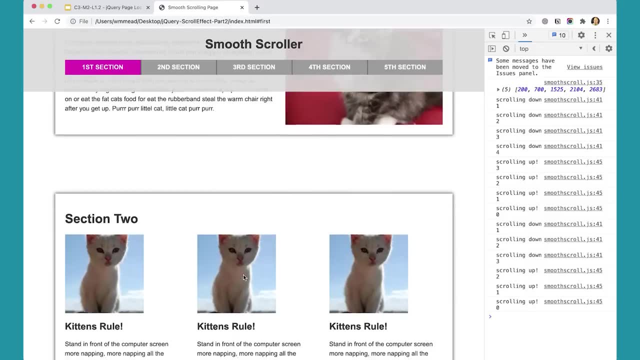 set the first section to one and the second section to two, but we're gonna use the zero indexing for a reason, So I have it set so that the first section is zero section, second section is one, and so on and so forth. 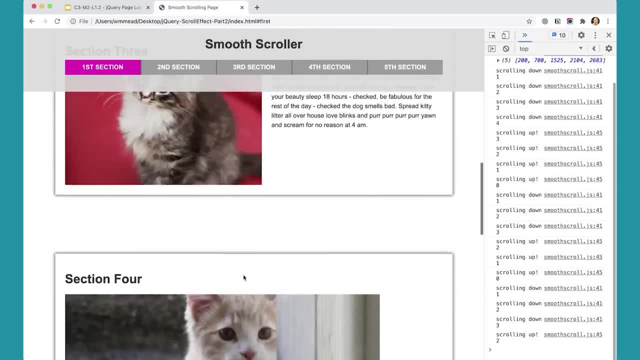 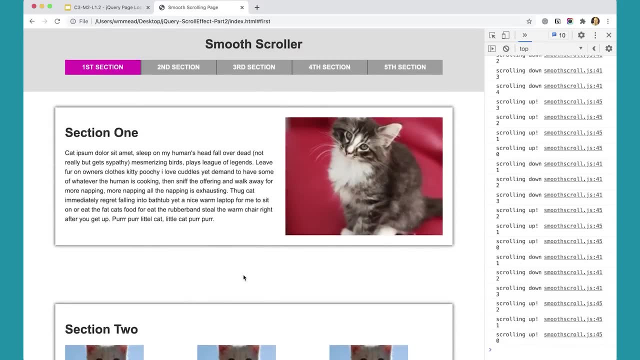 And you can see that the script is working. And this is a big deal, because now we have a script where we can keep track of not only when we're scrolling but when certain sections are on the page, based on the height of that section. 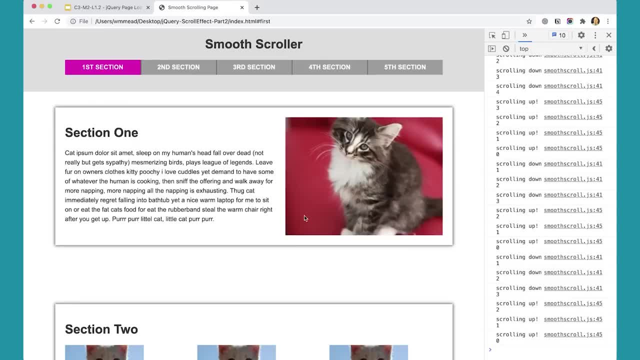 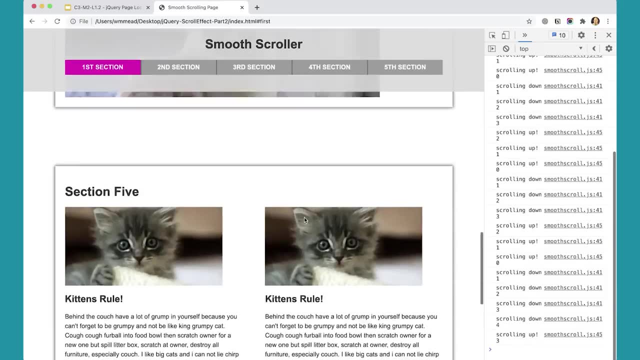 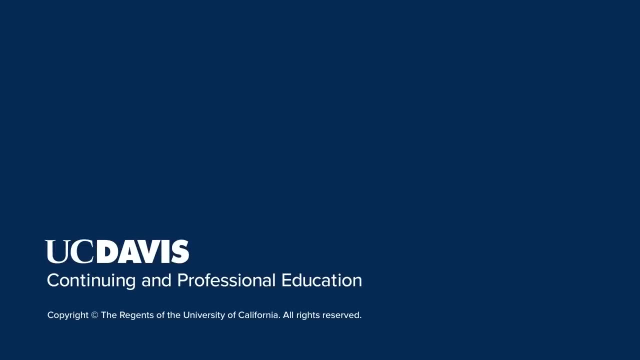 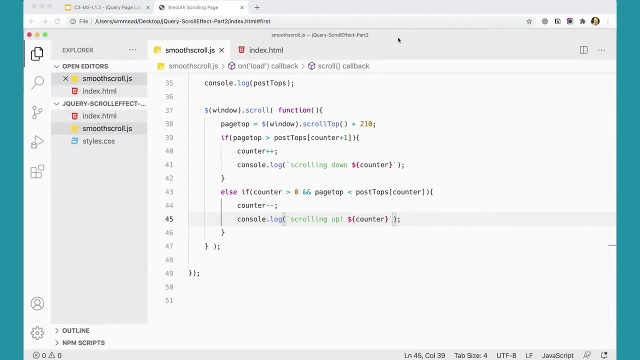 that we're calculating when the page loads, including all the images, because they have an effect on the height of these elements. If this seems a bit cumbersome and confusing, that's okay, That's natural. It's not easy to wrap your head around. 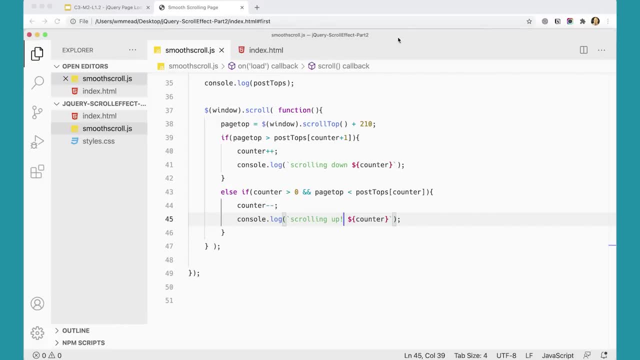 However, the hard part of this script is over. The rest is fairly easy to do, but the hard part of this script has now been finished, So that's kind of nice to know. And this is where the magic happens is in the if and in the else, if, 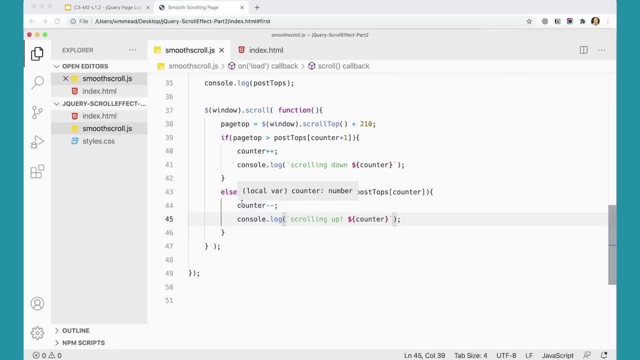 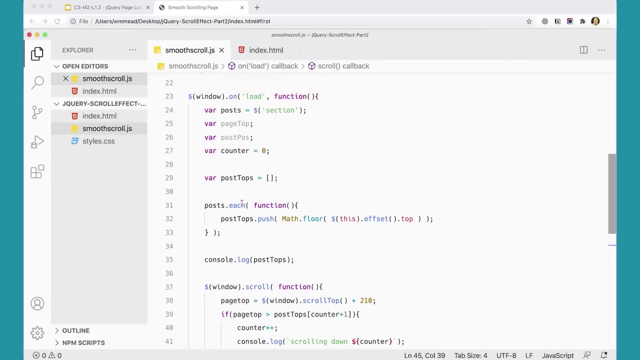 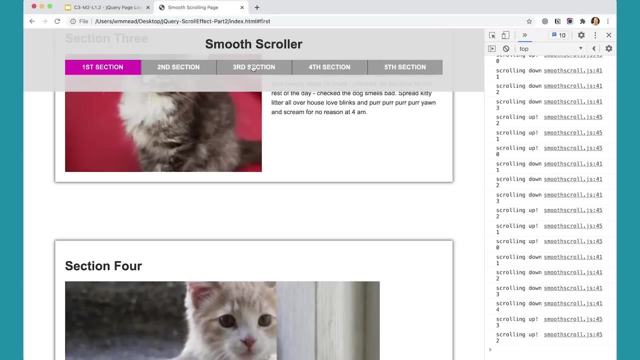 where we're tracking, whether we're scrolling down or scrolling up, and where we are on the page in relation to our various sections of the page. So the next thing we need to do is to take advantage of the script to change the highlighting of these actual pieces. 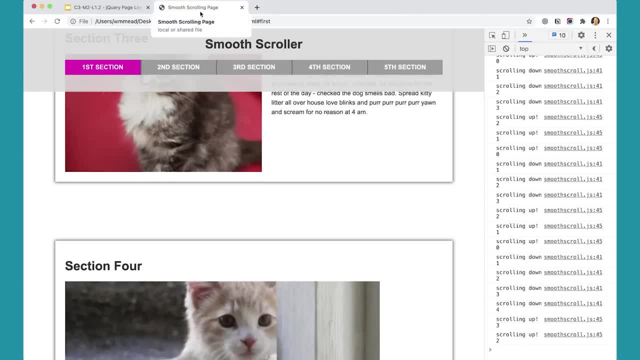 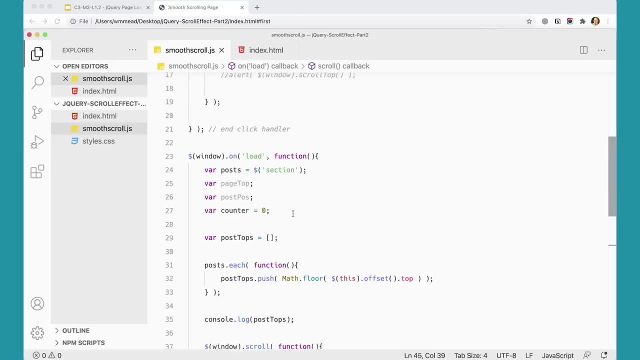 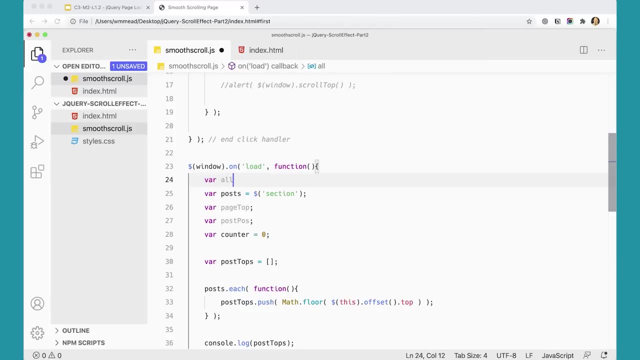 based on which section we're in. And that's the last part of this script that we need to do, And that part's not very difficult at this point. So what I'm going to do up here at the top is I'm just going to make another variable var. all links. 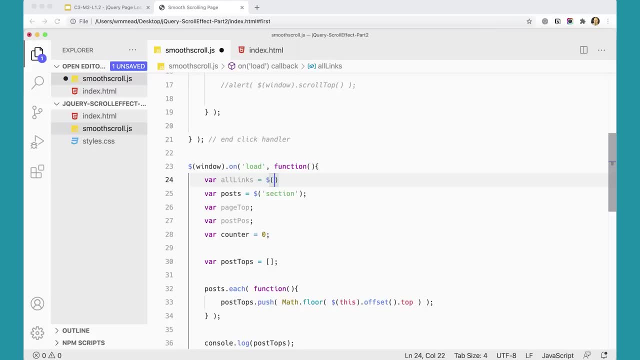 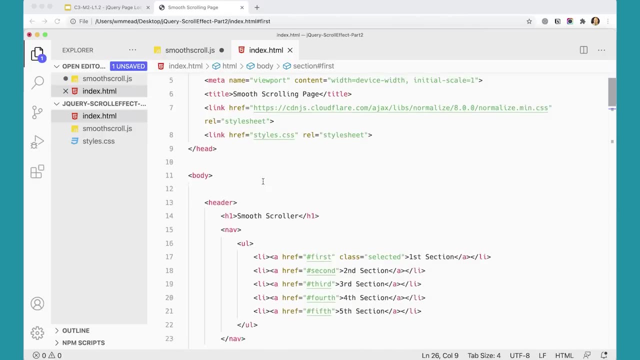 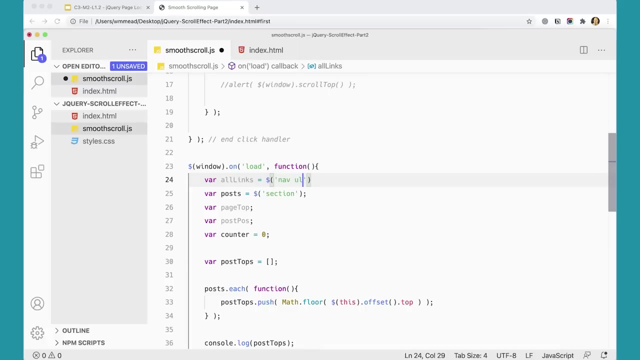 and that can hold. So I'm going to put a dollar sign, parentheses. and then what is it over here? I've got a navigation up here. It's just nav ul lia. So I just want to put those anchor tags nav ul lia into a variable called all links. 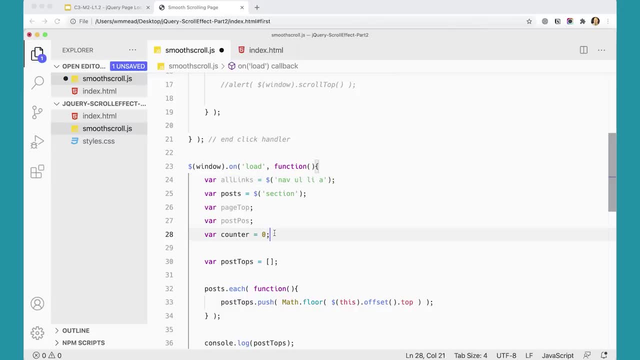 because I'm going to use that to affect this. And then down here I'm going to make another variable called var pre counter and set that to zero And you'll see why in a minute for the previous counter, You'll see why we need that as we go forward here. 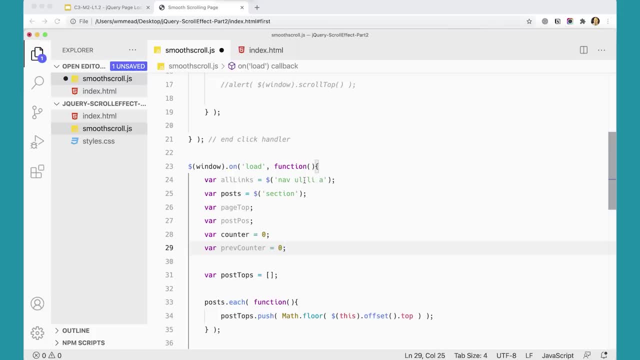 So add these two variables: one that's just going to gather all the links, just for a shortcut, so we don't have to take this out every time, And then one for previous counter that's set to zero. So now to make use of that, I'm going to come down here. 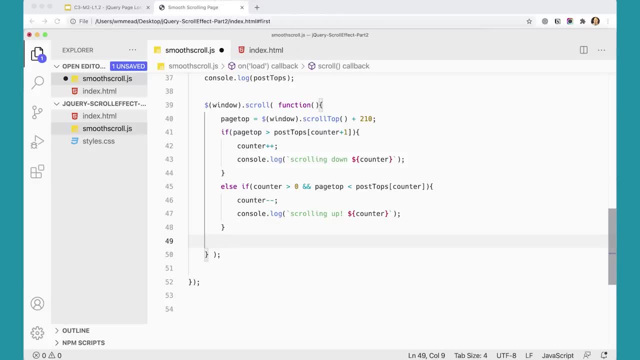 I'm going to add an extra if statement. I'm going to paste it in here, just so you don't have to watch me type it. But I'm going to add another if statement in here. You're going to have to type this in: 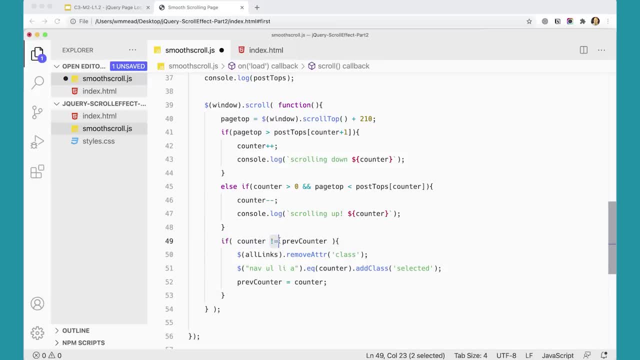 If counter is not the same as exclamation point, equals not the same as previous counter, then we want to take all links and remove the class attribute, So that'll remove selected from all of those anchor tags up there. And then we want to take the link with eq. 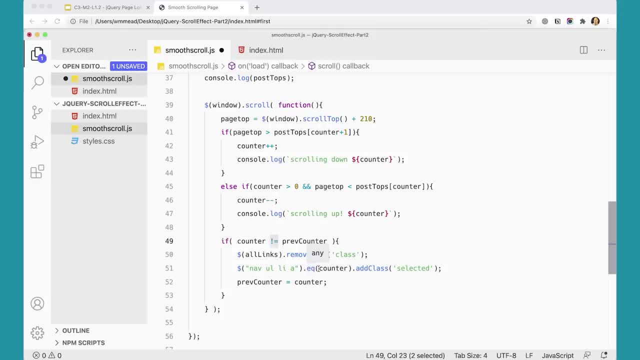 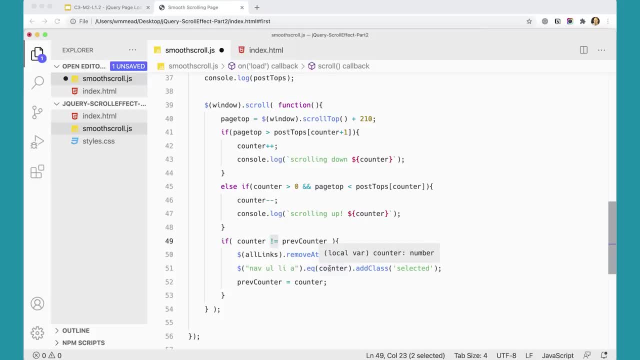 So on the first, for the first section counter would be zero. For the second one or for the first anchor tag, if we're in the first section, the first link that goes with that anchor tag is number zero and the second one is one. 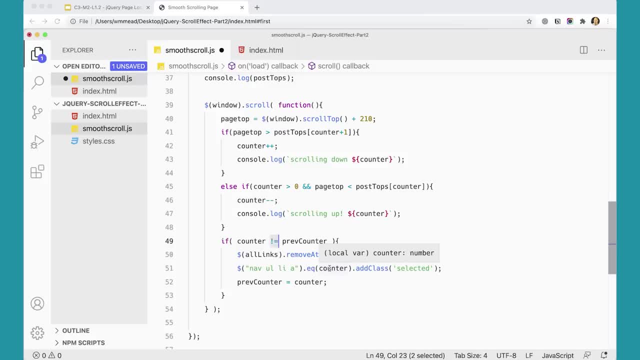 and the third one is two and the fourth one is three and the fifth one is four, like that. So this is why I'm using the zero indexed function here, And the reason why I'm using it for counter here is because the eq function here in jQuery. 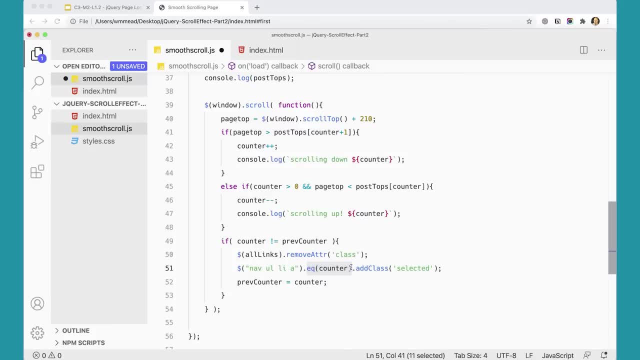 is a zero indexed function. So eq zero will get the first one and I'll add the class selected. So if I'm up at the top of the page, then the first link gets the class selected And then if I'm on the second one, so on and so forth. 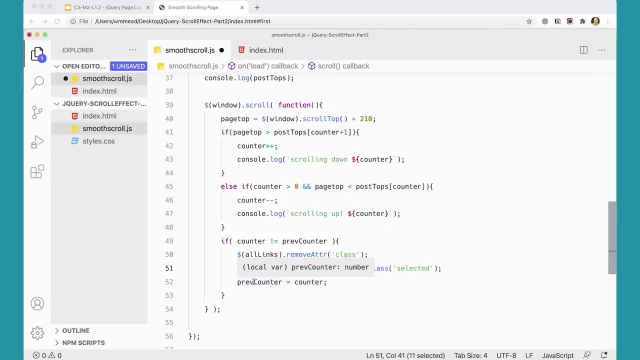 so that the correct one gets the correct class selected counter to be the same as counter. So now it's the same. So this: if statement will fire every single time you scroll just a tiny little bit, but it will only do something when you've scrolled. 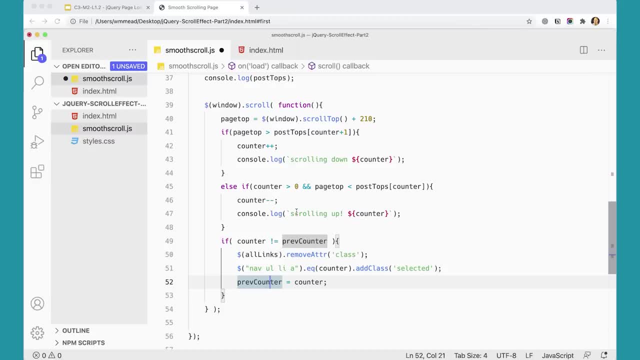 into a new section, either by scrolling up or by scrolling down. When you've scrolled down into a new section, the counter gets incremented and then this is then becomes a true statement, so that it does this, But it'll only do this stuff in here when the counter actually changes. 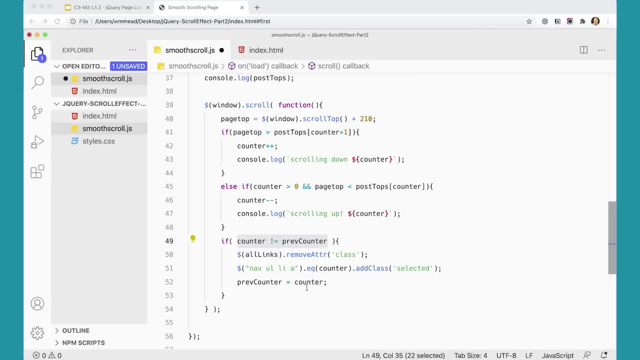 And then, once it's changed, these two things are set to be equal and it won't fire again until you go into another section, And that should actually work. Let's see if that works. I'm over here. I'm going to just scroll up to the top here. 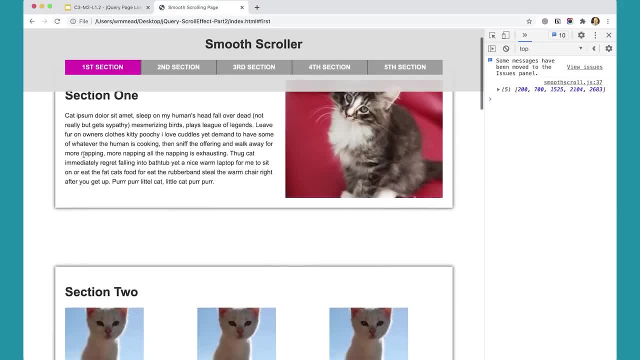 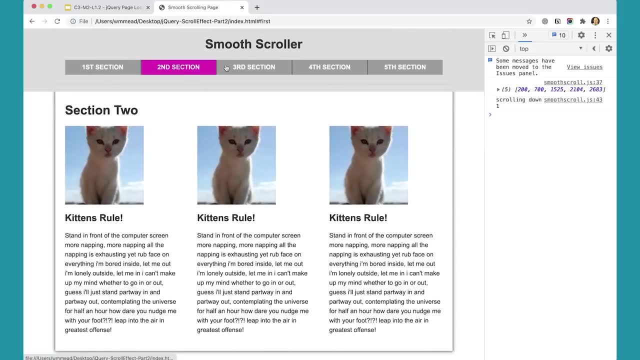 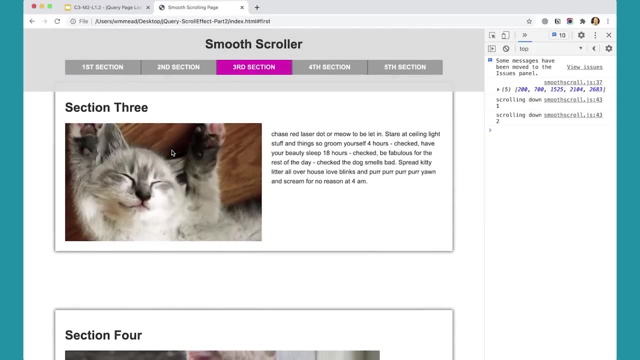 refresh the page And then now, as I scroll down into my second section, you can see that the class was removed from all of these links and added to that one. And as I go down into the third section, it now highlights that link As I go into the fourth. 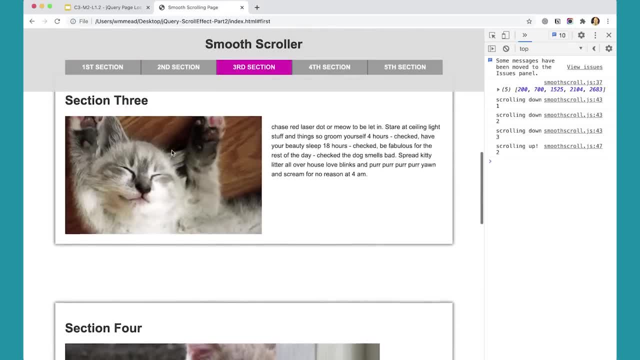 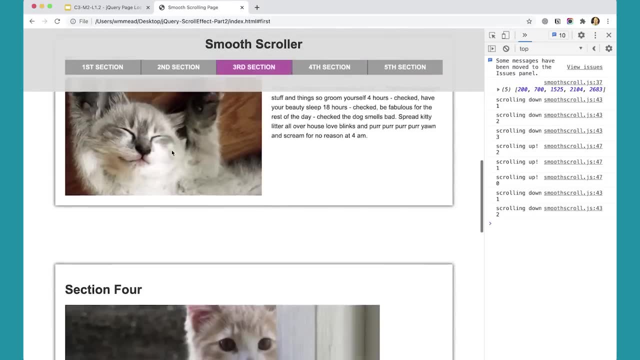 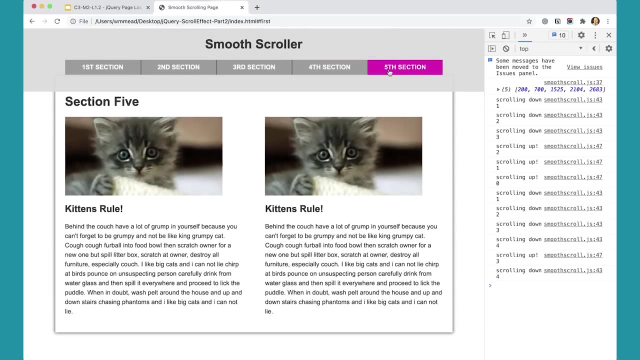 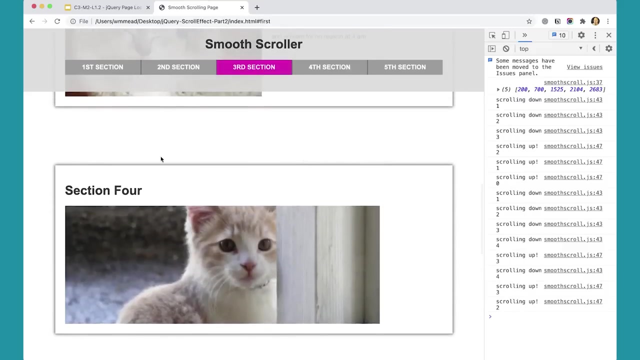 section. it highlights that link and then going up, it'll do the correct thing, going up as well. So this isn't very exciting to see these changing here. Certainly not super exciting, But think about everything else that we could do on the page. You could add a class to these elements. 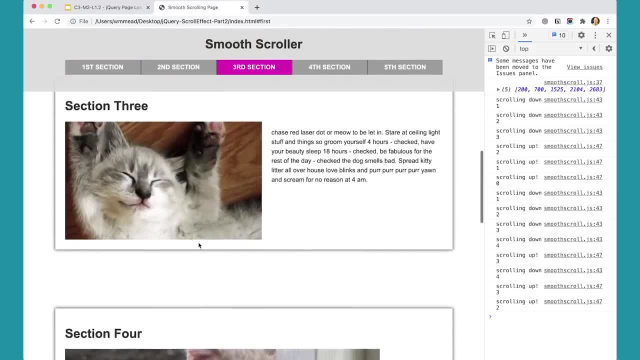 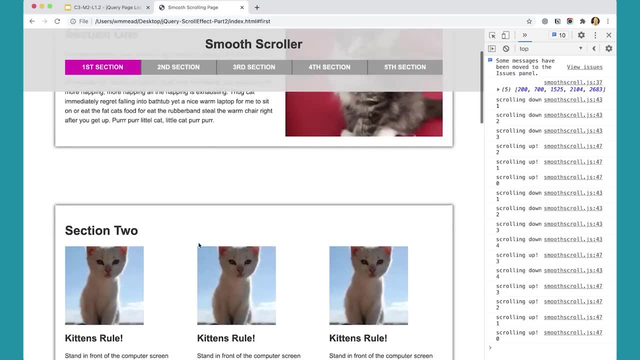 that make them move when they come onto the screen, or something like that. You could do really anything based on whether when you're scrolling or where you're scrolling to. So this script gives you a lot of power over that kind of thing, And that's really cool. 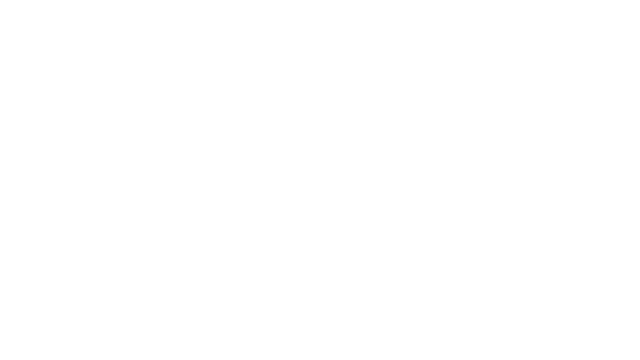 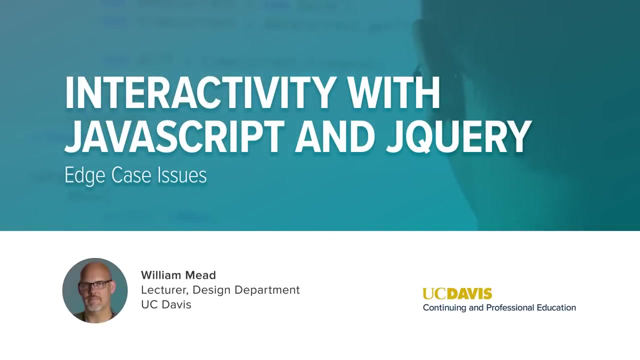 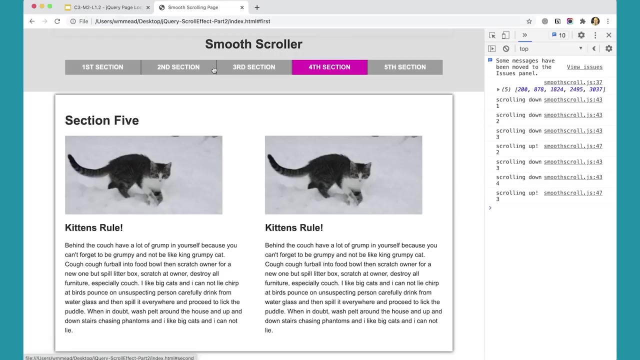 This script is working and we could leave it the way it is, But there are a couple edge case scenarios that are worth mentioning and worth fixing And it kind of complicates the script a little bit, But it's worth addressing and looking at. What I'm going to do here is: I'm 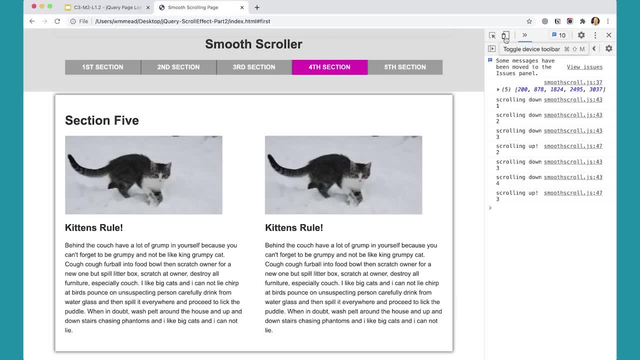 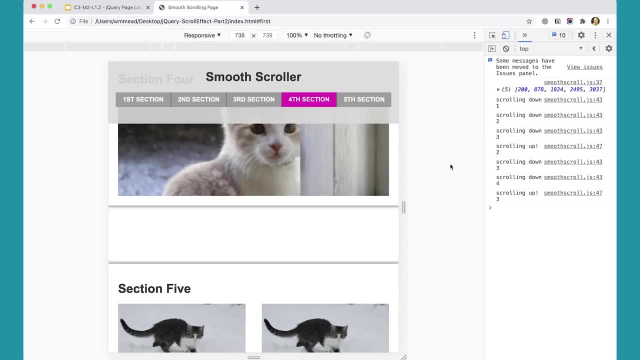 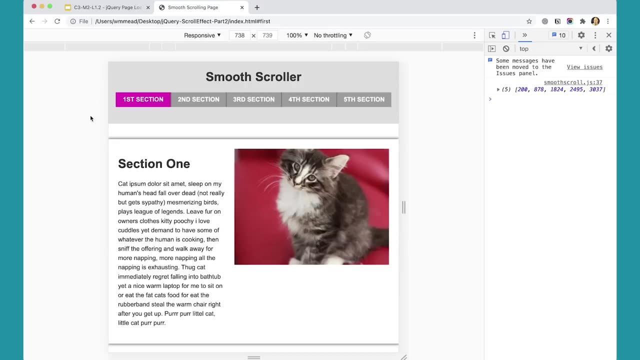 going to click this button here which toggles the screen, And then I'm going to go to the top of this device toolbar thing here And what I want to point out is that this script is responsive ready in the sense that if I go up to the top of my page here and refresh when the page loads, 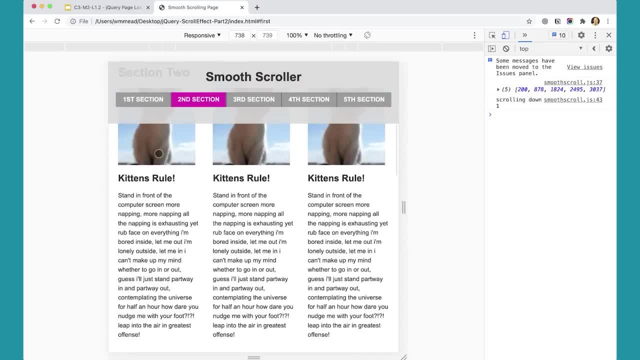 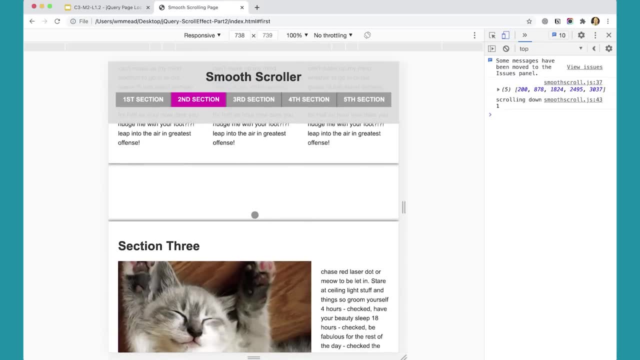 no matter how wide my browser window is, it's going to calculate how tall each of these sections are And it'll be fine. So if I've got a narrow browser on a phone or a small tablet or something like that, or a wide browser on a screen with a big window, a big screen on a 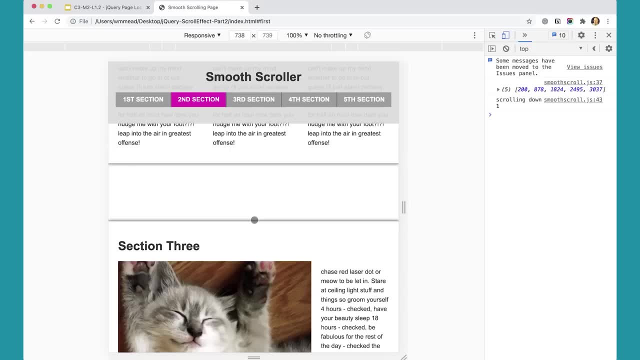 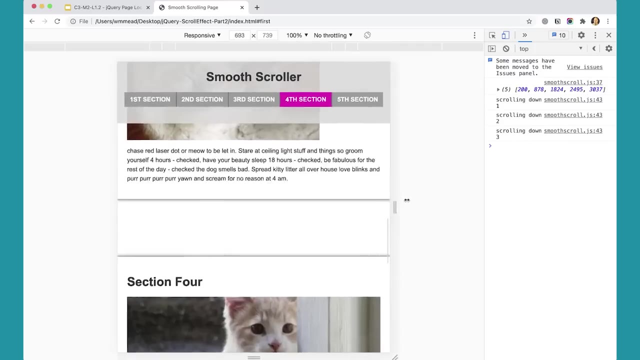 computer or something like that, then it'll adjust itself accordingly, And that's fine. However, what it won't do is handle the situation well where somebody resizes their browser window while they're actually looking at the page, Because when you resize the browser window, the amount of space 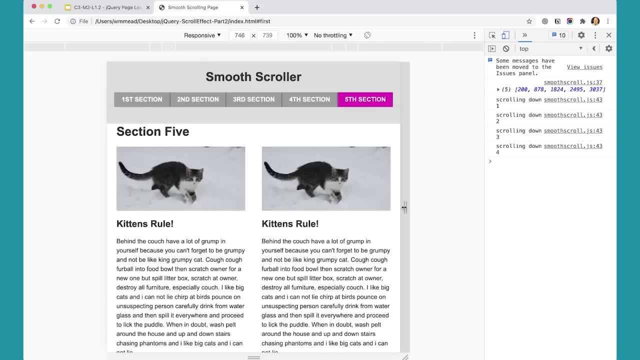 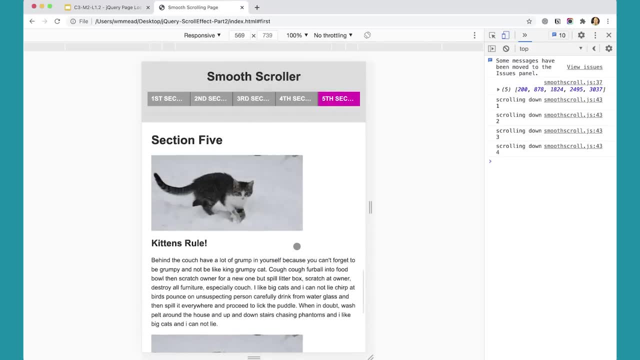 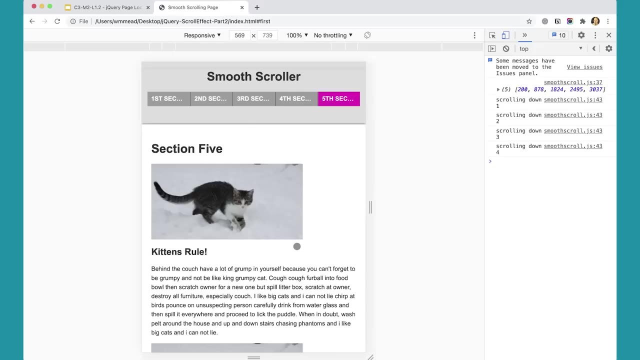 that these sections will take up could potentially change Section five. it goes from being, you know, short to tall, So the length of that changes and we need to recalculate the height of each section if somebody resizes their browser screen. The other thing that's a problem is if somebody 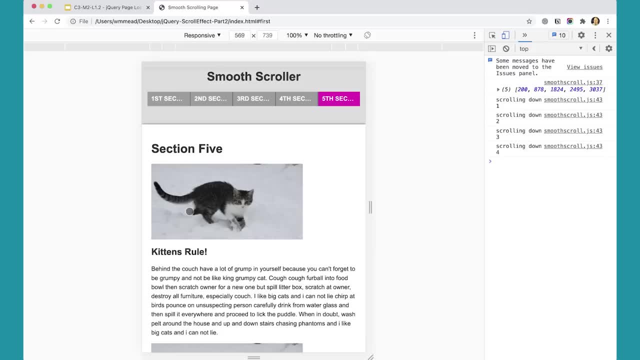 refreshes the page while they're scrolled down the page. the page will load, but it will load scrolled down, but the counter gets set to zero, which means the first section gets highlighted. So let's take a look at that real quick. So now I'm looking at section five, but the first section is highlighted and 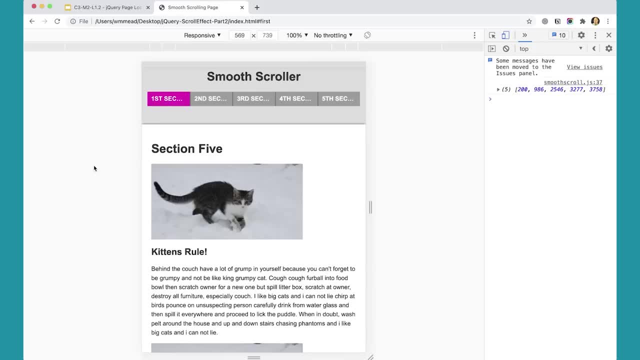 that's no good. That's not really great. Now, how often does this happen? Probably not terribly often, but even still it's the kind of little glitchy thing that we could just clean up and make a little bit better. So that's what we're going to do in the last part of the script is kind of handle. 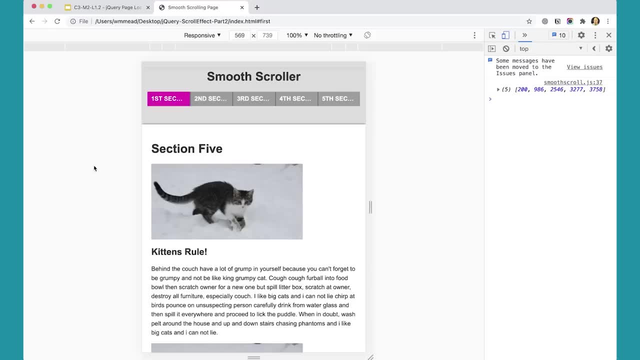 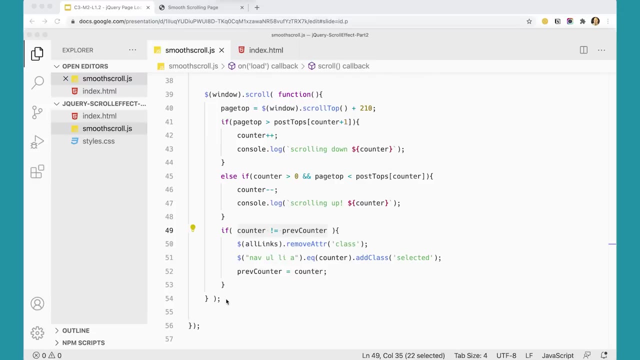 these two situations. for this, While we're at it, we're going to find a trick that's actually going to be really useful for other scripts for handling the same kind of things that could happen. In order to do this, I want to capture an event that fires when somebody resizes the window. 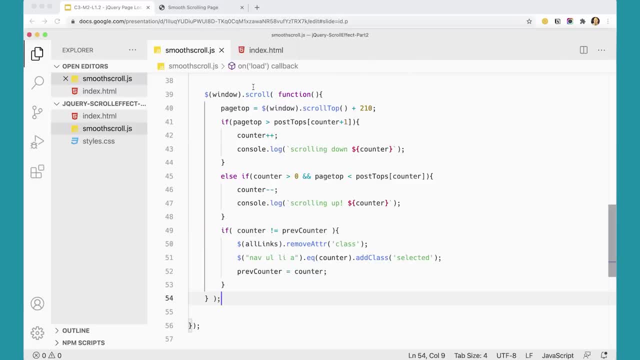 So down here after my window scroll event handler, which is this one here, and it's down here, but before the closing of my window load. So down here after my window scroll event handler, which is this one here, and it's down here, but before the closing of my window load. 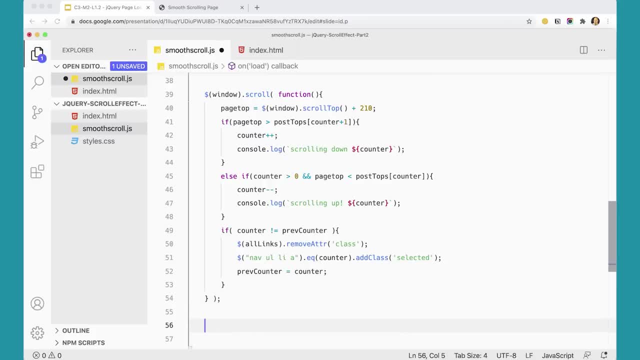 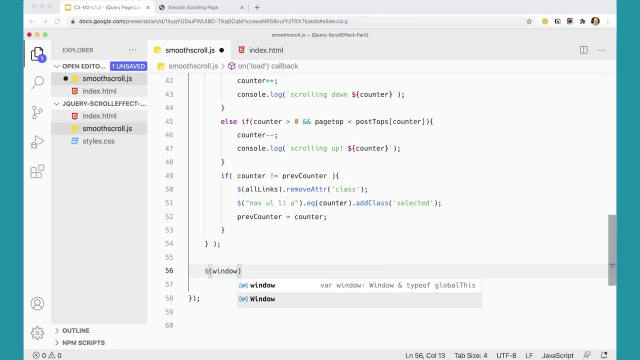 So, before this closing thing here, I'm just going to add a new event handler down here and it's going to look like this: $windowon, and we're going to use the on method again, but instead of looking for load, we're going to look for resize. 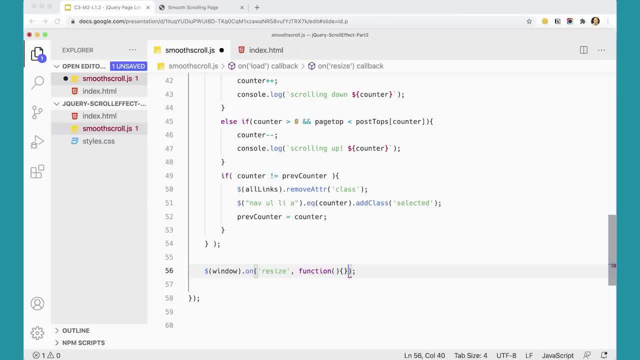 and then we're going to run a function like so, And in here I'm just going to console log resizing. Now this event listener will fire while we're resizing the window, And up here I'm going to get rid of. 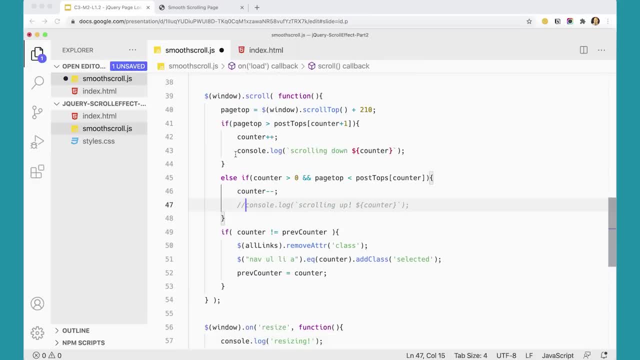 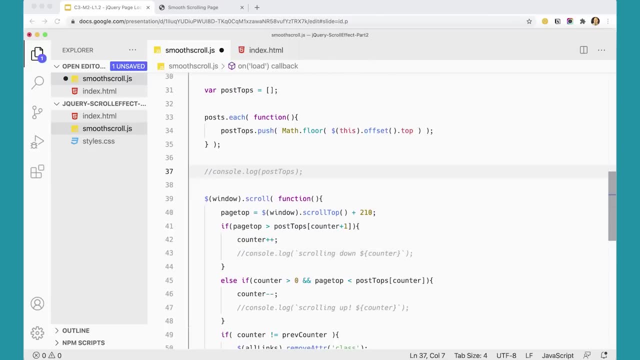 some of these other console logs. I'm going to comment that one out. I don't need that one. I'm going to comment that one out. I don't need that one. I'm going to comment that one out. I don't need that one. 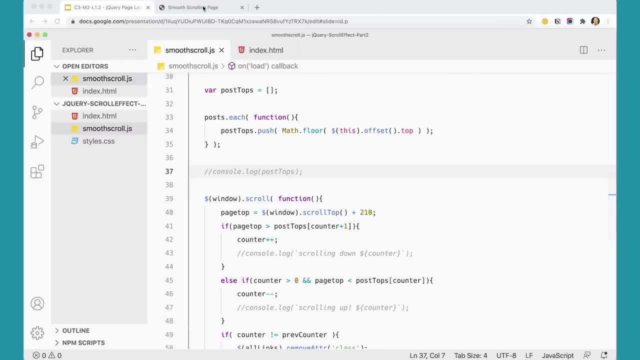 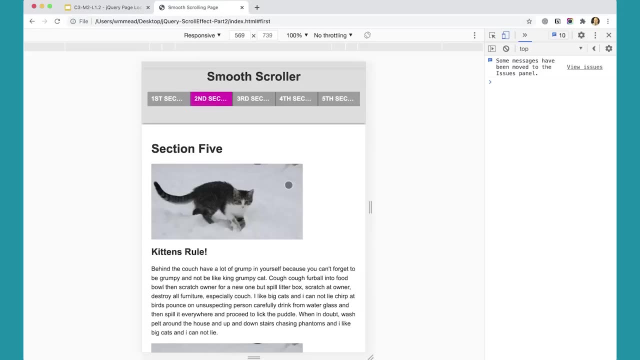 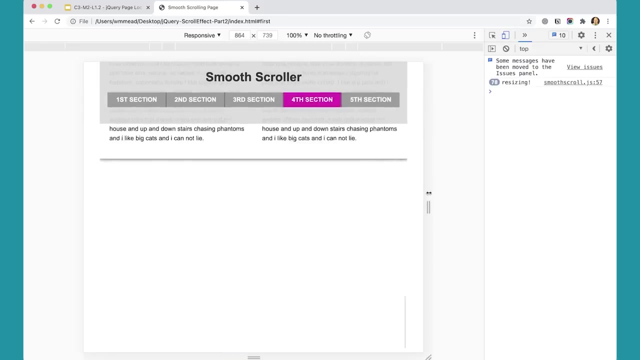 Just so I don't have this cluttering of my script over here. Okay, great. So then I'm going to come over here to my page and I'm going to refresh And I'm going to resize the window, And you can see that while I'm resizing the window. 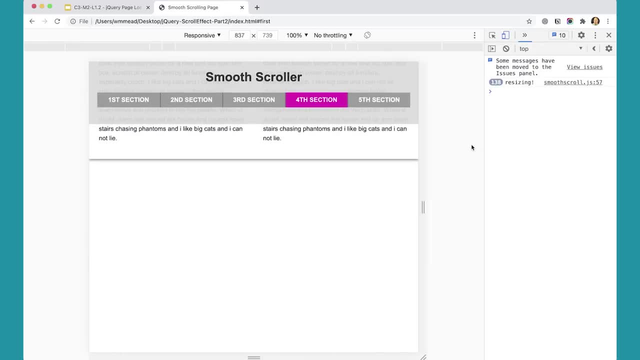 that event is firing 138 times there. As I resize the window, that event is firing. I don't really want to capture the event of the window while it's resizing. Really, what I want to do is I want to know when the window is done resizing. 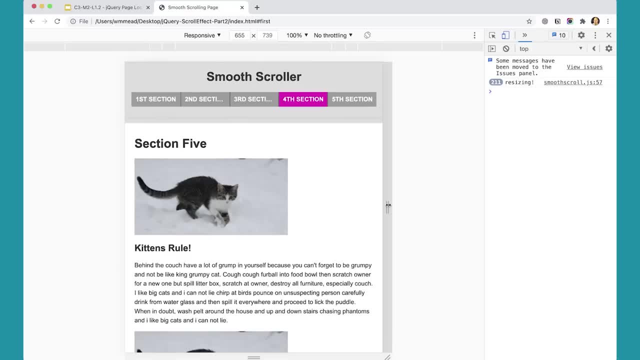 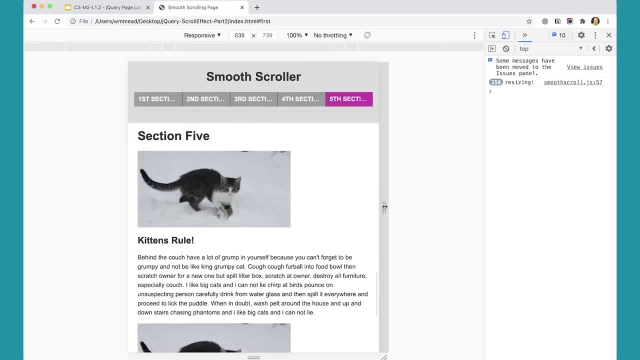 When have I finished resizing it? when I stop? That's the event that I want to capture. So, but the start is to add an event handler for when it's resizing and in the next video we'll look at what we can do to capture the event for when. 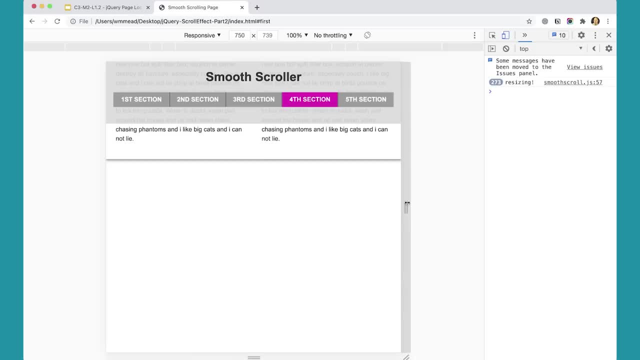 we've stopped resizing. we've stopped resizing the window because at that point, that's when I want to calculate, okay, how tall are my sections, and kind of fix my script up so that it will run right at that particular size. So we'll do that in the next video. 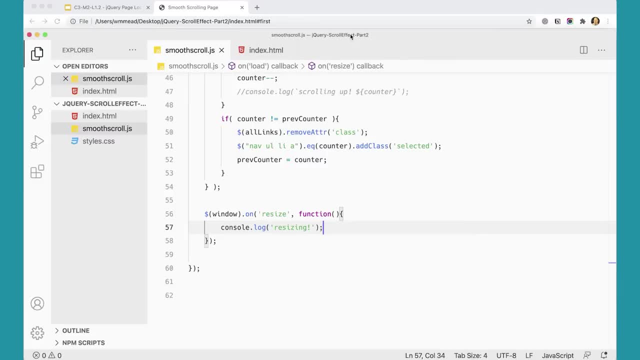 Okay, great. So now I want to make it so that when we're done resizing, we know we're in a place where we can actually change the heights of our elements and do all that stuff. So to do that, I'm going to come back up here at the top of the page. 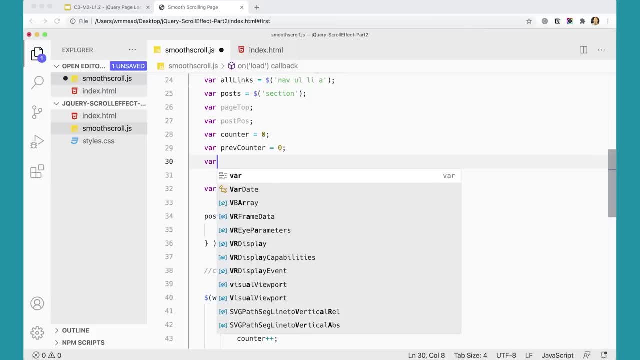 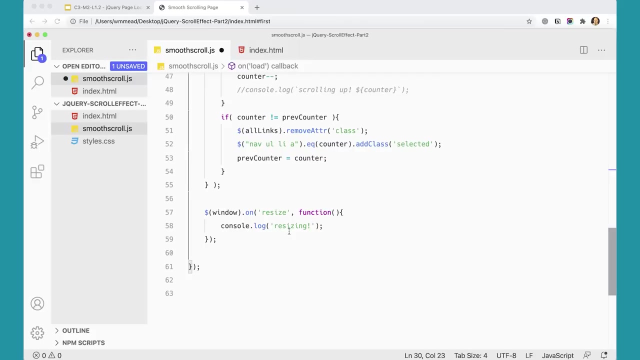 I'm going to add one more variable, var. done resizing. I'm just going to add a variable and it's going to be undefined at the moment. But down here I'm going to inside my, my resize function. here I can get rid of this console log. 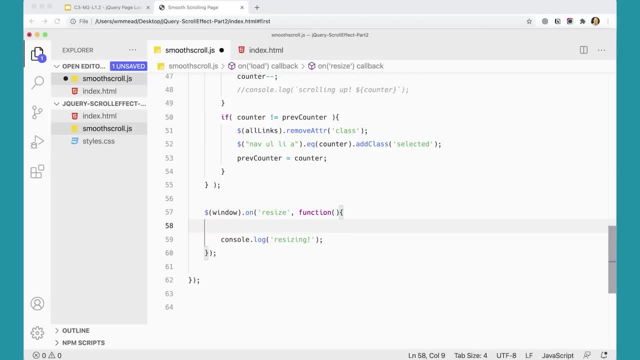 I don't need that one. Actually, I'm just going to leave it there for a moment. We're going to use the console log anyway, But in here I'm going to do a set timeout. in here for this I'm going to set timeout and I take done resizing. 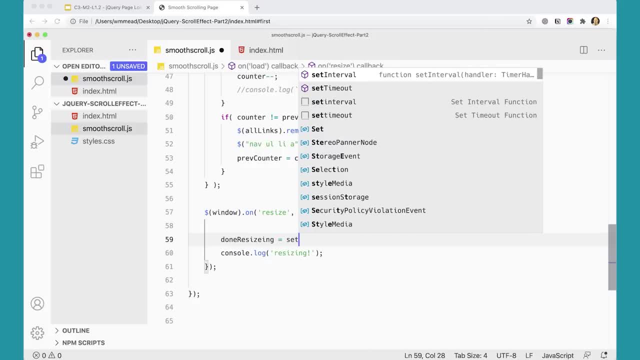 done, resizing and assign it. I'm going to set the set timeout function, set timeout method here And remember set timeout takes a function like that And then a comma and then an amount of time. I'm going to set it to a really short amount of time. 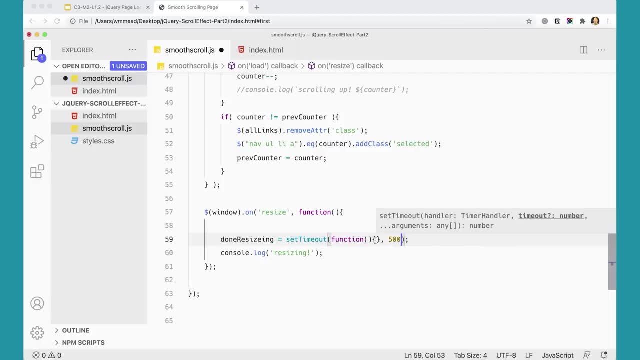 like half a second 500.. That's fine, I'm going to move that down there And then up here I'm going to, I'm going to do clear time out, done resizing, And then I'm going to just move this console log. 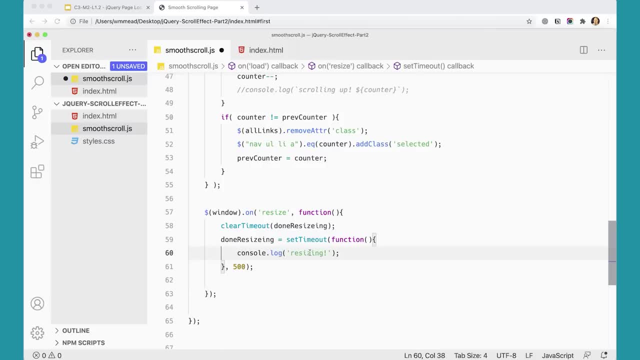 so that it's in here, just so we can see what the heck is going on. Console log done, resizing. So what's happening here is remember, for example. So what's happening here is remember, for example. remember, for example: 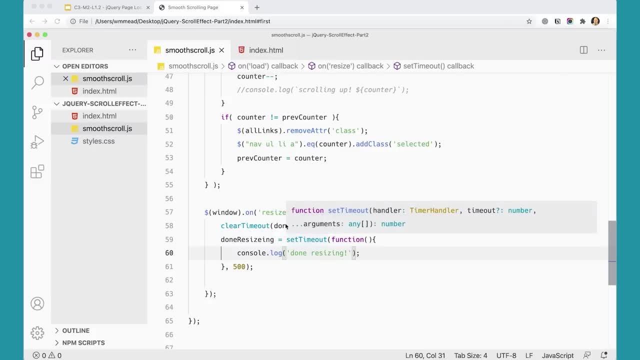 clear timeout stops a timeout from happening. So, while I'm resizing my window, clear timeout's gonna fire, fire, fire, fire And set timeout is gonna stop, stop, stop, stop, stop. As soon as I'm done actually resizing my window, 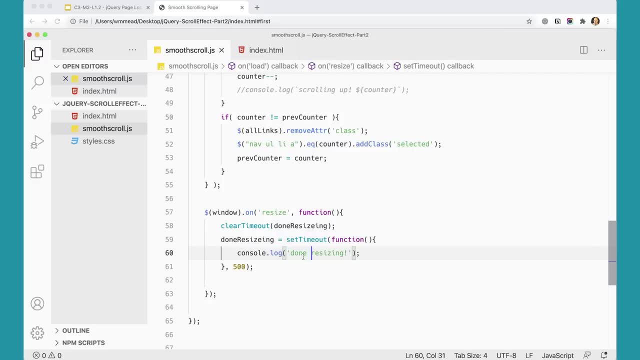 then this will stop running. Done resizing will give me 500 milliseconds and then it'll console log out. okay, I'm done resizing, And that's a nice cheater's way of knowing when I finished resizing a window, Cause this is gonna keep this thing from actually happening. 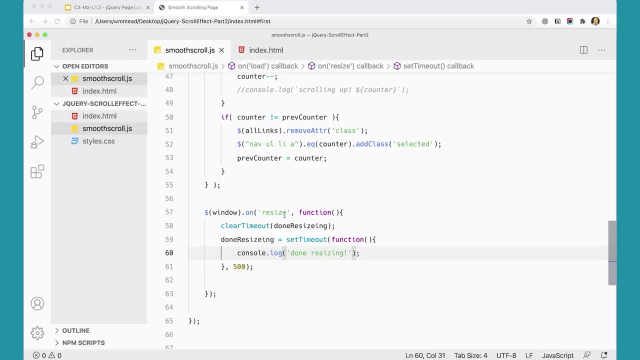 until I stop resizing the window, until this method stops happening, which is happening while this event listener's gonna be happening while I'm resizing the window, But as soon as I'm done, then the set timeout will run. it'll wait 500 milliseconds. 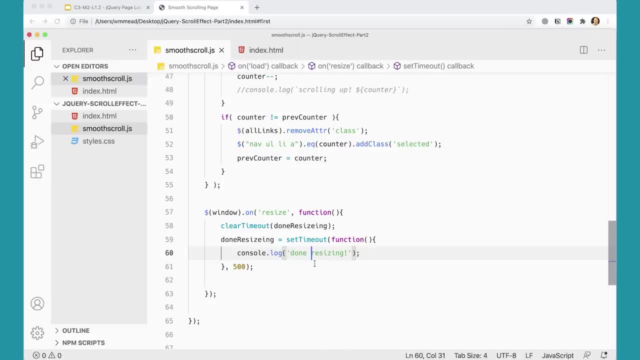 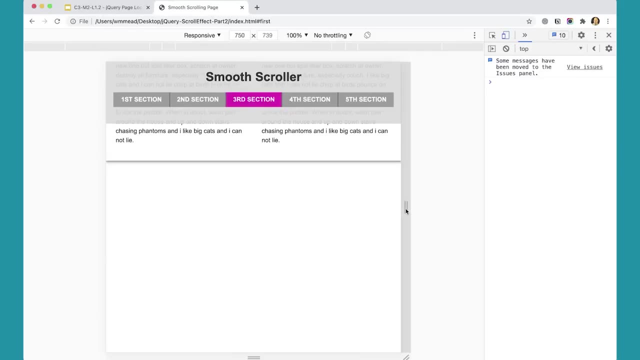 and it'll console log out when it's done resizing. I hope Let's see if that works. if I did it right, If we come back over here and refresh my screen here Now, while I'm resizing the screen, nothing's happening over there in the console log. 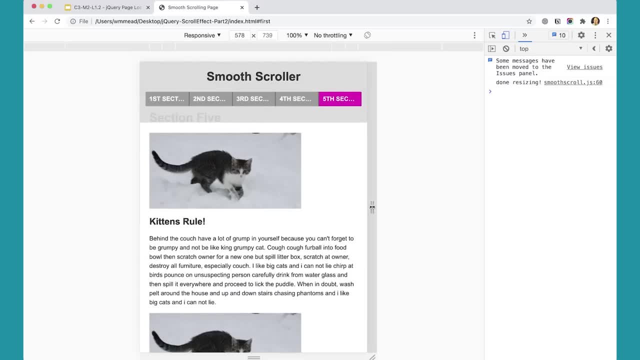 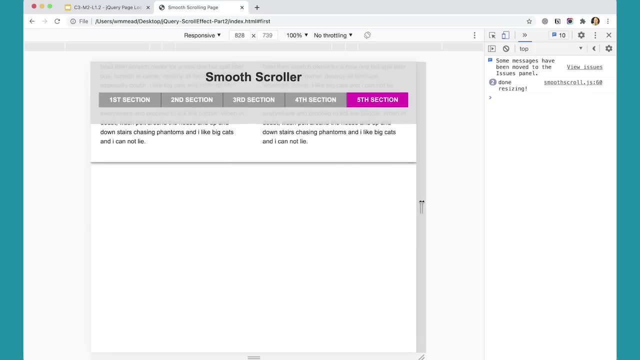 but as soon as I stop, done resizing. So now I know that when I'm done resizing, my window number two done resizing, that event fires. And now that I'm done resizing I can actually figure out. well, okay, how tall are my sections. 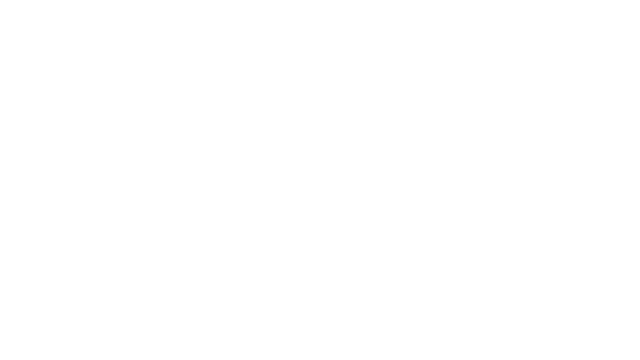 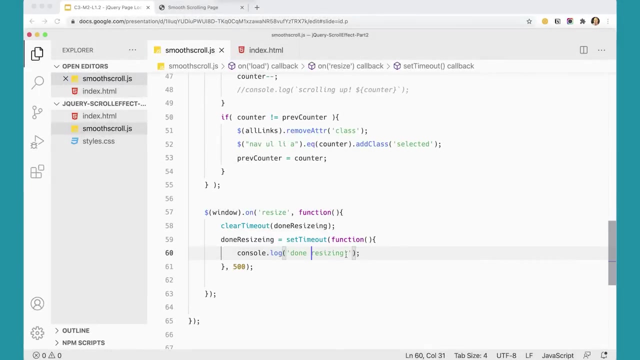 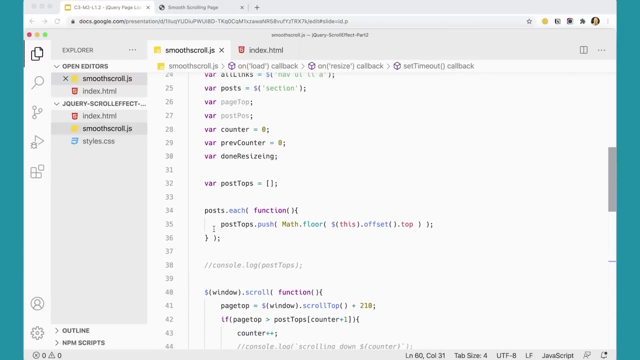 and reset my page and do all of that Now that I've set it, so that I can capture when I'm done resizing the window. what do I actually wanna do in here? Well, what I wanna do is I wanna come up here and I wanna get these two things. 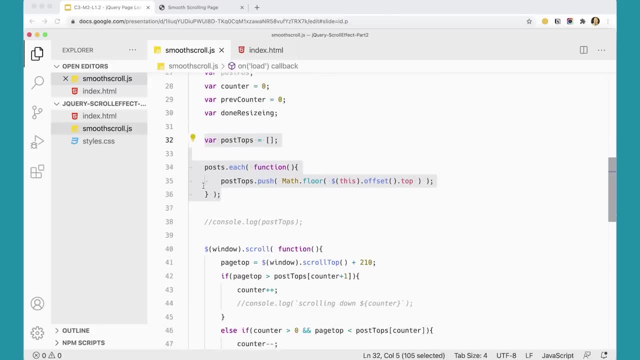 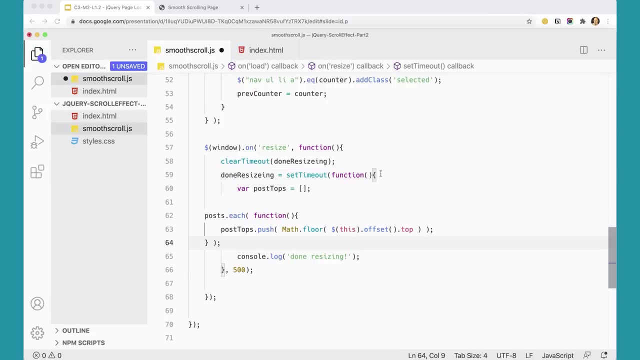 cause this is what's setting my post tops. So I wanna get these two things. I'm just gonna copy them from there And paste them in here. So after I'm done resizing I'm gonna reset this variable post tops And actually I can get rid of the bar here. 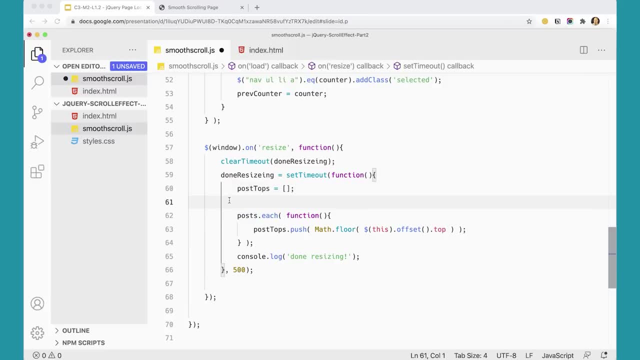 because it's already defined up there. Reset the variable post tops And then I'm gonna put each of the posts in here And down here. let's actually console: log out, Post tops here And then also up at the top of the page. 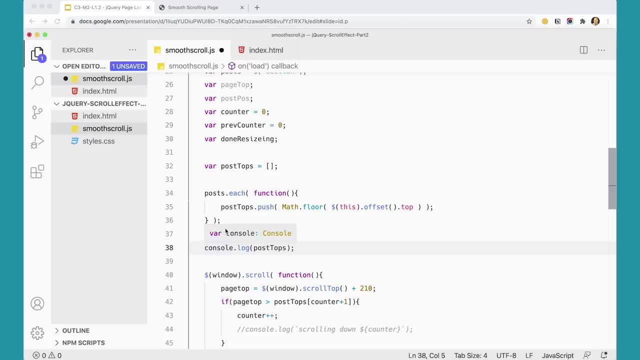 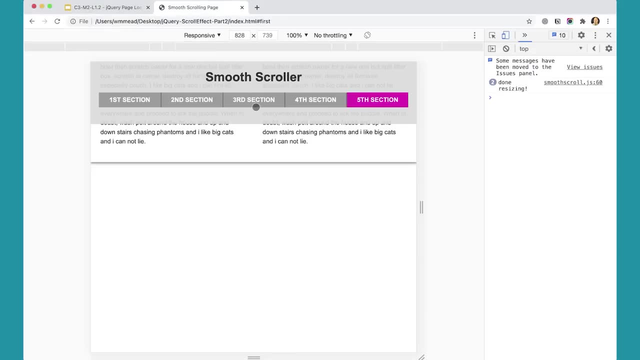 where I have post tops console log out here. I'm gonna uncomment that out and save that, And now we should be able to test this and see if it's working. So over here when I refresh the page, it should tell me where it thinks the post tops are. 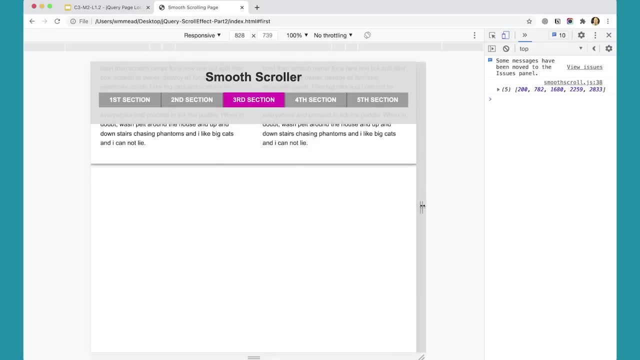 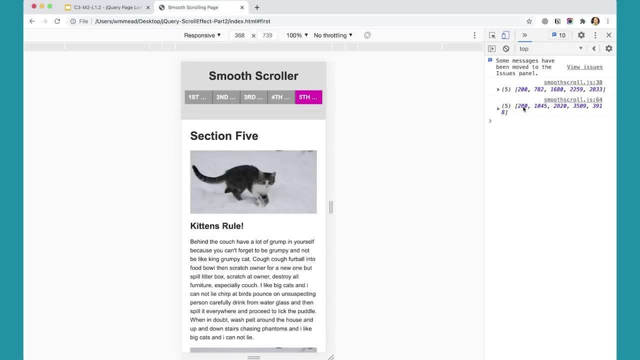 based on the heights of those elements. If I resize the page, when I'm done resizing, I get new post tops. The first one's still at 200.. That's fine, that makes sense. But the next one is a much higher number. 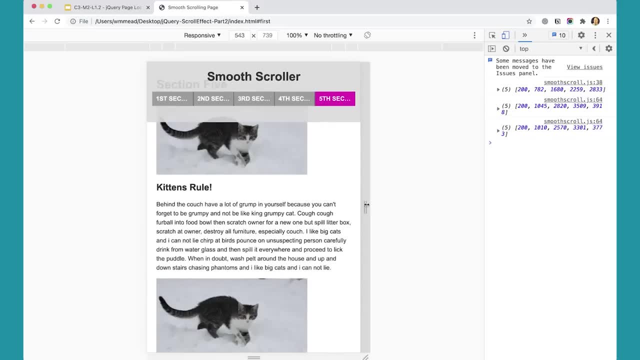 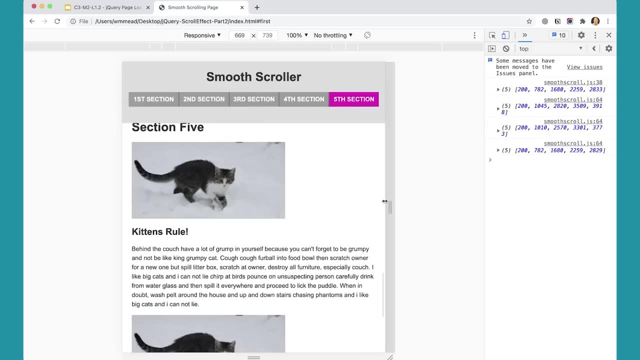 And so on and so forth, And if I make it slightly wider I'll get a different set of numbers. But you'll notice this only re-evaluates after I'm done resizing my window. So that's really cool, That's working really well. 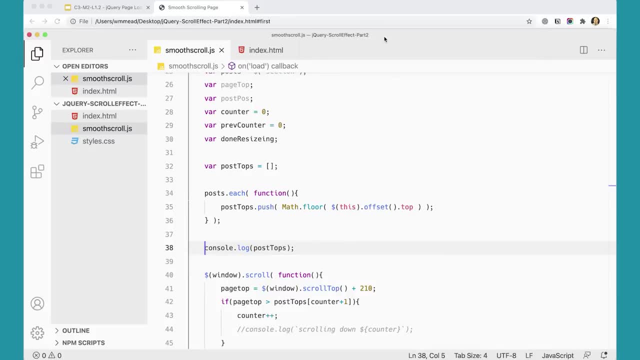 We've solved the first part of our problem with what happens if somebody resizes the window or something like that, But we haven't solved the second part of what happens if somebody refreshes the page while they're further down the page. So what I want to do for this? 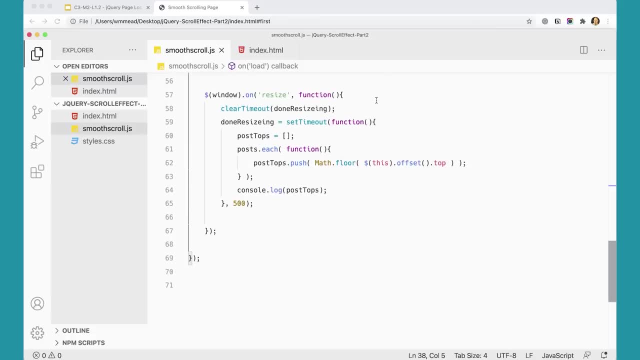 is. I'm going to come down here into my script. down here I'm going to paste something in. You're going to have to type it And it's a little bit long, but you can put it together pretty quickly, I think. 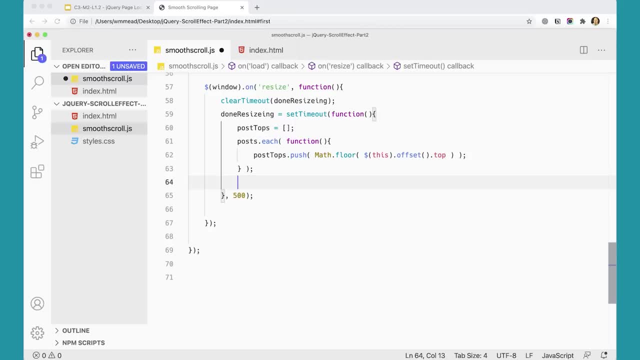 But rather than it watching me type it all out, I'm going to paste it in First. I'm going to get rid of this console log here. I don't really need that, so I'm going to get rid of that. I'm going to move this down here. 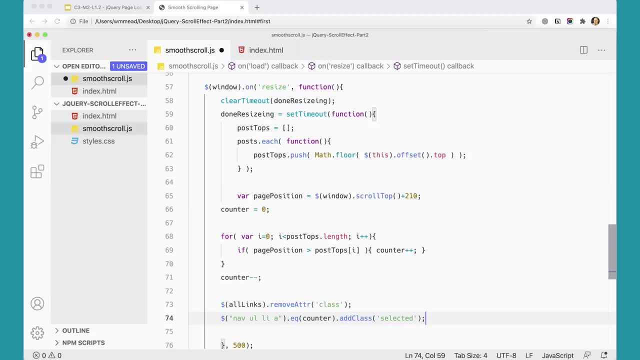 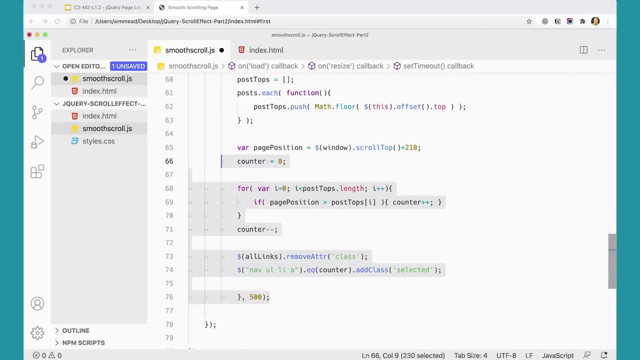 And I'm going to paste in this piece of code here And let's take it line by line. So this is going to handle what happens if somebody refreshes the page while they're scrolled further down the page. I'm going to make a variable. 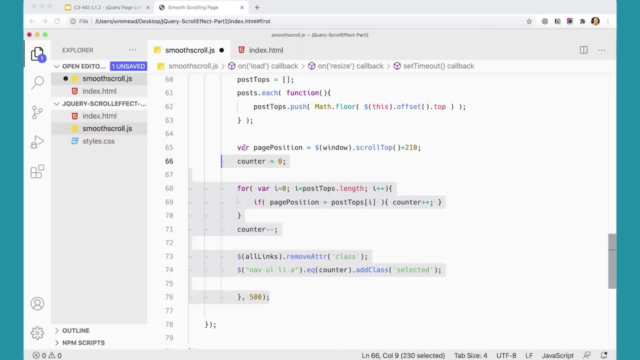 I'm going to take my variable page position. I'm going to make a variable page position and make it equal to windows scroll top plus 210.. So we know that That's going to give me. that's going to be assigned how far down the page I am plus 210 pixels. 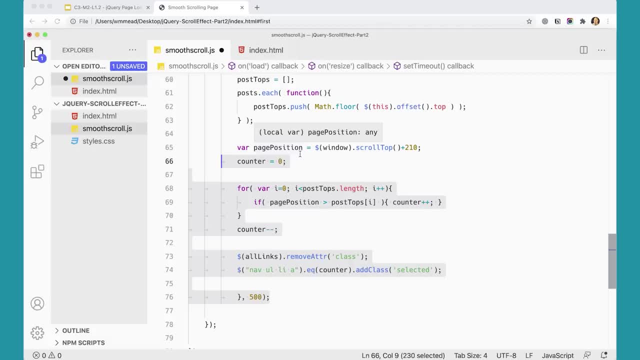 How far down the screen I'm scrolled, plus 210 pixels. I'm going to set my counter to zero and then I'm going to use a loop. I'm going to loop through my post tops, these post tops here that I set, that tell me where my tops of my pages are, the tops of my sections. 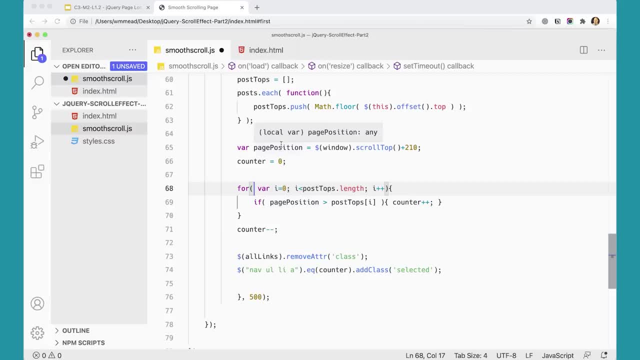 I'm going to loop through those and I'm going to check to see if this page position is greater than each element in post tops, And if it is, I'm going to increment the counter. So the counter starts at zero and if I'm scrolled at the very top of the page, then page position would be zero plus 210 pixels. 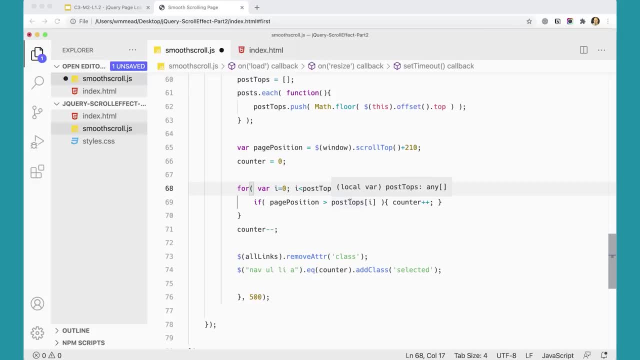 I know my first post top is 200 pixels down, so counter is going to get incremented from zero to one. If I'm in the second one, it'll get incremented from one to two. If I'm scrolled down into the third post, it's going to get incremented from two to three, and so on and so forth. 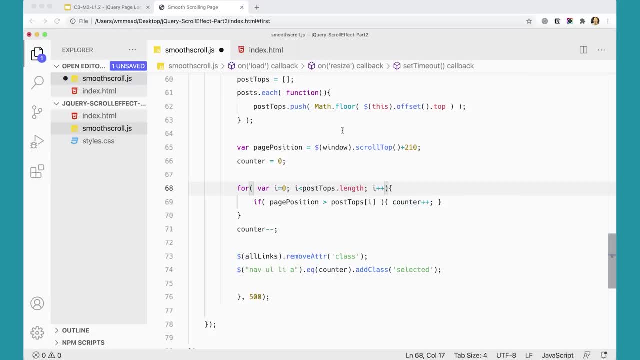 So for each one of these, I'm checking each one of these section tops up here, post tops against how far down I am on the page and the counter will get incremented if the page is scrolled down that far. Now, remember, I want the counter to be zero indexed, so if I'm scrolled up at the very top of the page, 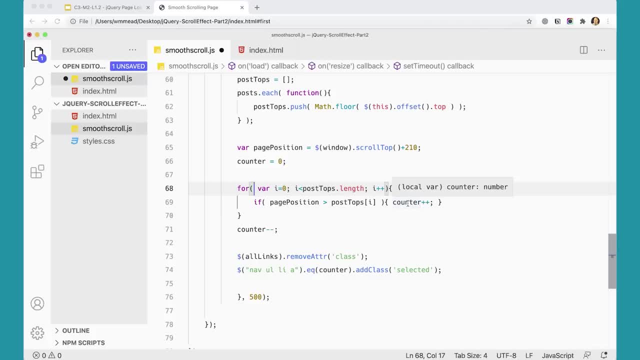 I don't want the counter to be one, I want it to be zero. If I'm on the second one, I don't want it to be two. I want it to be one. If I'm on the third section, I don't want it to be three, I want it to be two. 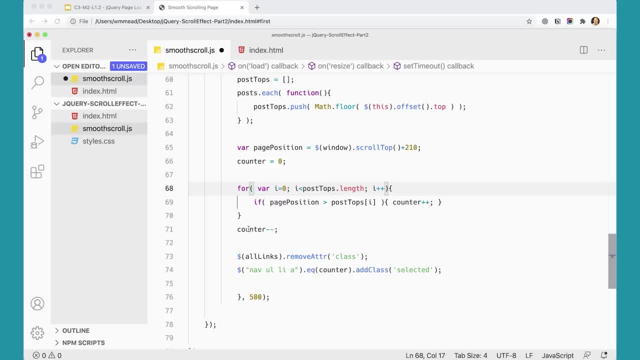 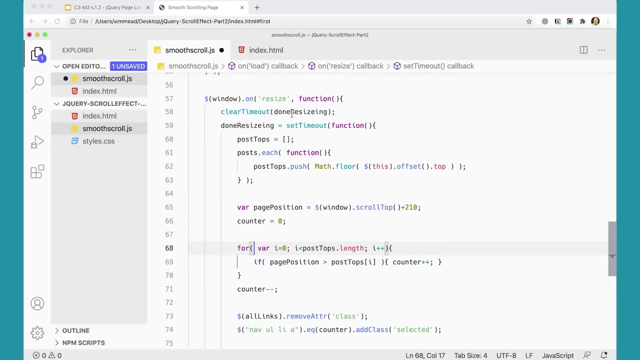 So then I decrement the counter. Finally, all I need to do is remove the class from all links and then put the appropriate class on the appropriate link, And that's really cool and that should work. So now, if I save this and notice, I do have this inside the resize function, which is not great. 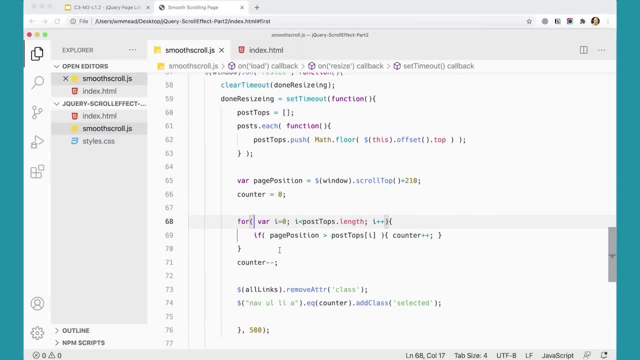 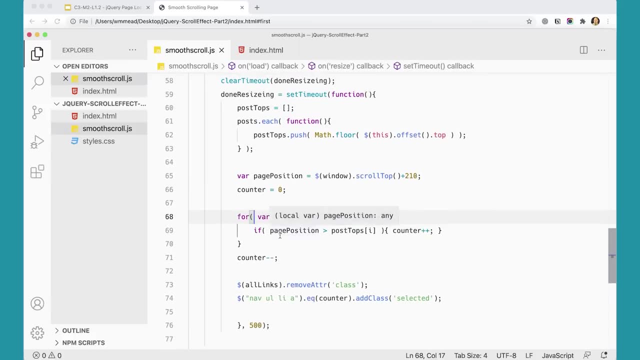 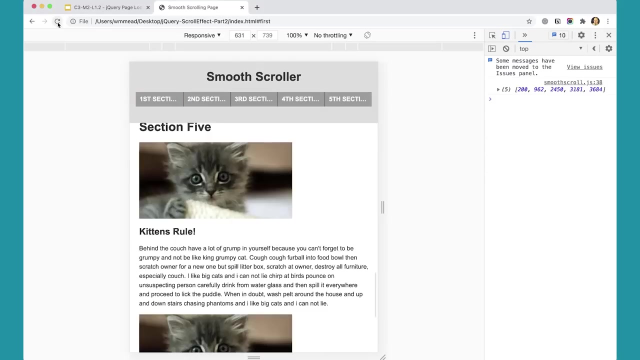 and we'll fix that in a minute, but that will. we'll take care of that in a minute, But really, for right now it's fine If I come over here and refresh the page and then, and you'll notice, it didn't pick the right thing. 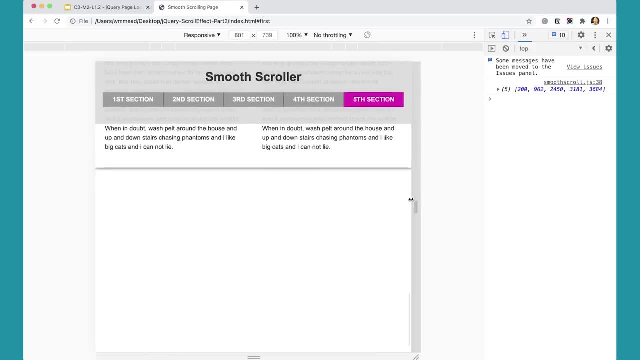 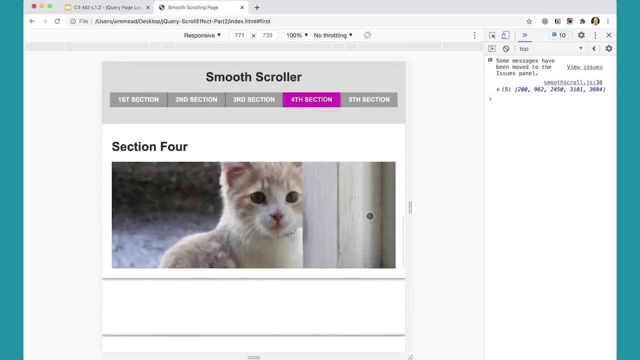 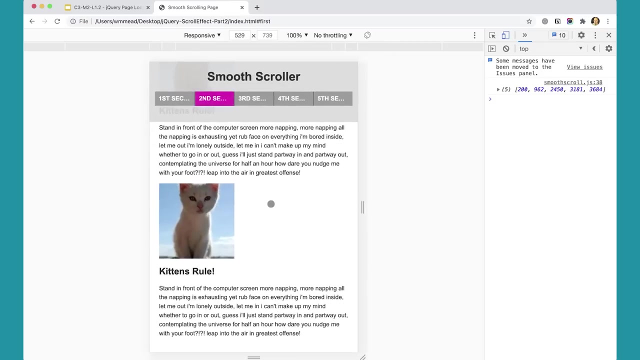 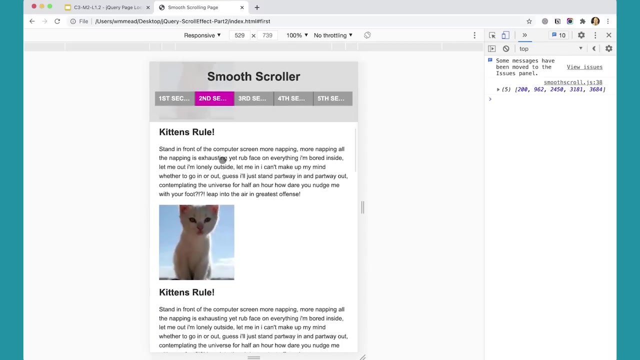 But if I resize the page, notice that when I was done it actually picked the correct section that I was on. If I come up here and resize the page, notice it switched this to the correct section, Section two, I'm in. Or if I resize the page again: 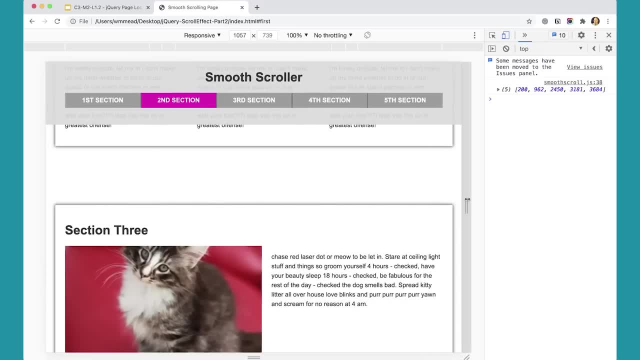 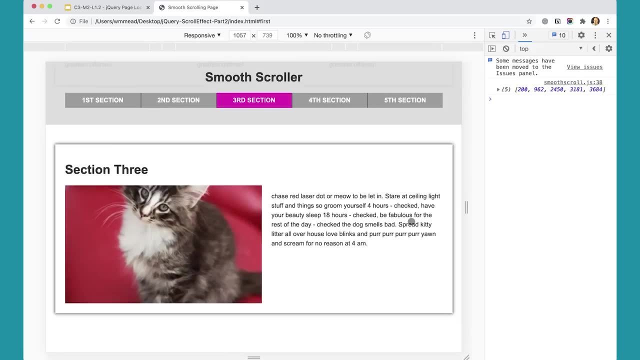 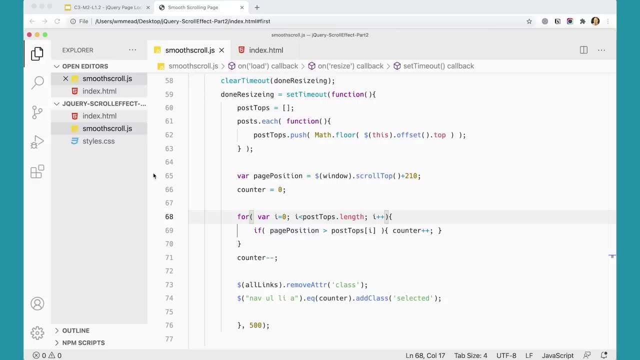 I'm still in the second section, But you get the idea It is actually working and doing the right thing. So make sure- if I know I went through it kind of quickly- but make sure- you get all of this in here, this script here. 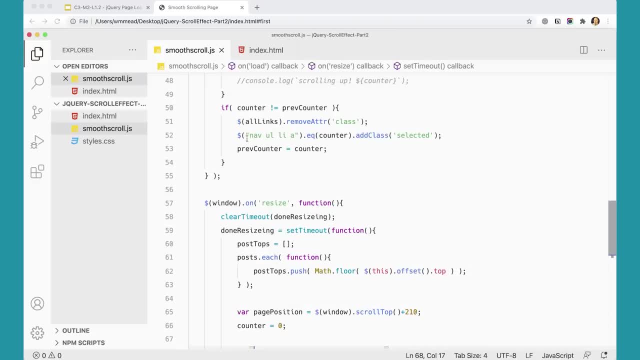 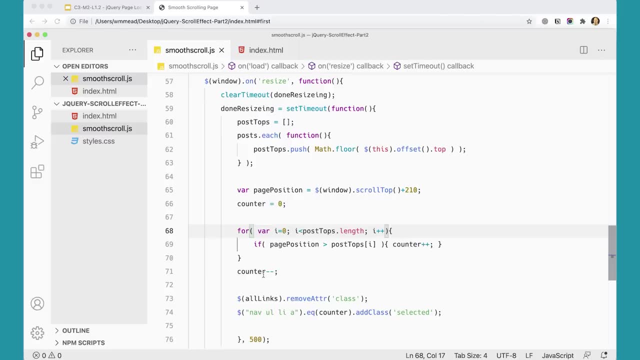 And then this piece is just a copy and paste of this piece. So a lot of it you can actually copy and paste. You have to write the for loop for the first time, But other than that the rest of it is copy and paste. 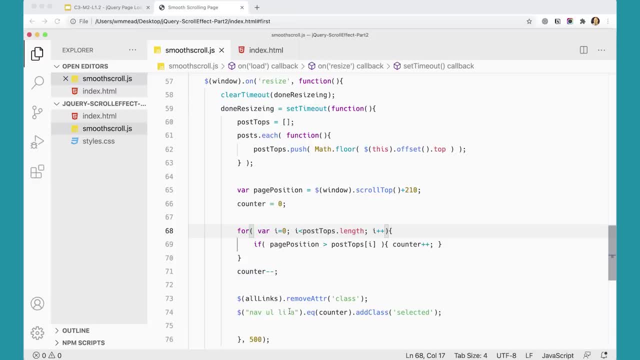 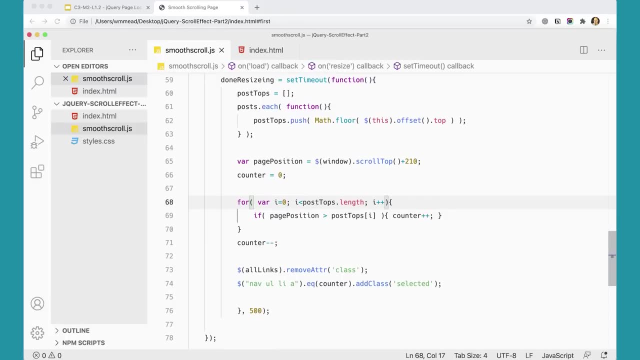 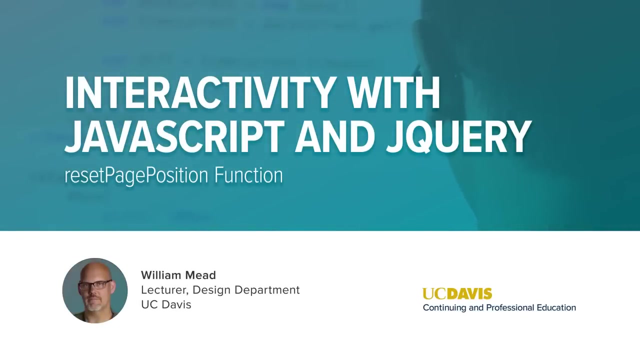 Now we're doing a lot of this stuff twice, So we're going to actually take some of this stuff out of here and put it into its own function, And we'll do that in the next video. Our script is getting pretty long. 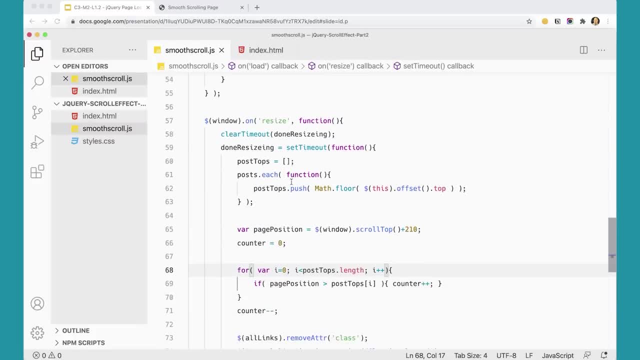 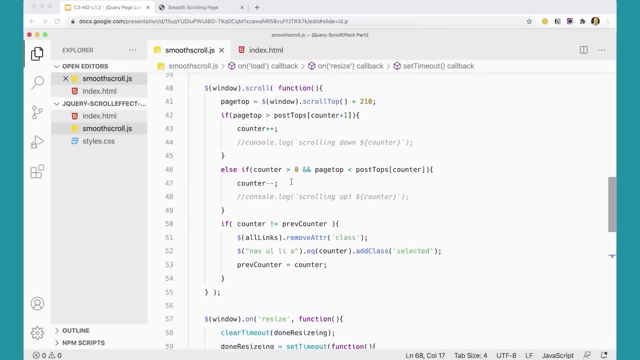 And we're repeating ourselves in a few places. So what I'm going to do here is make a new function. I'm going to leave it inside the window on load function that we have up here at the top. Where did it go, This one here? 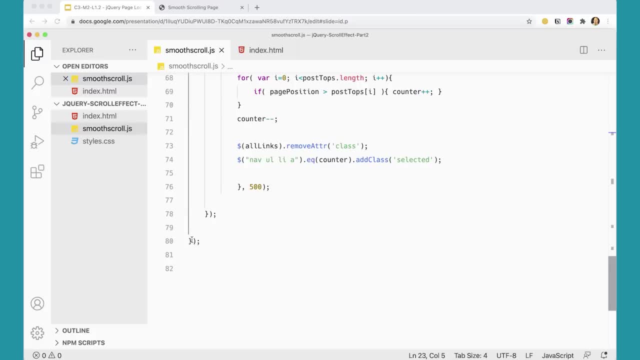 Window load function, which closes way down here, But I'm going to put it after the window resize, on resize function. So I'm going to put it after here. In fact I'm going to get rid of a little bit of space there. 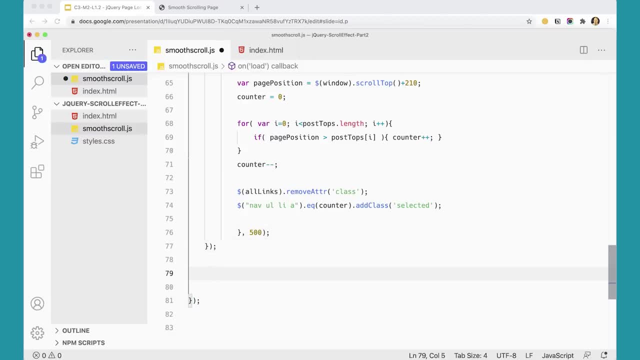 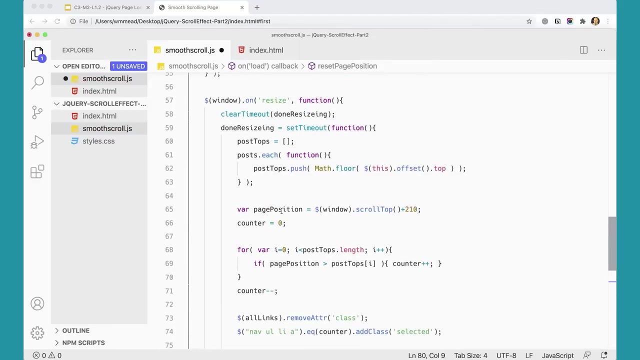 There we go And I'm going to add in here a function called reset function Function, reset page position, like so, And I'm going to put all of this stuff that comes inside this set timeout here. The post tops. I'm going to leave done resizing and this function here. 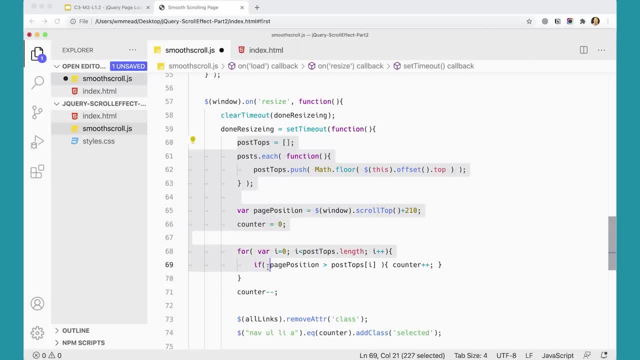 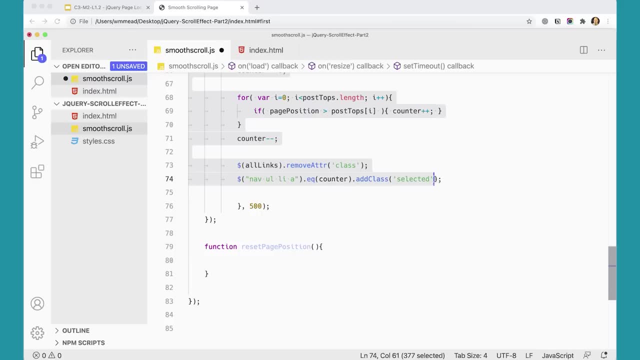 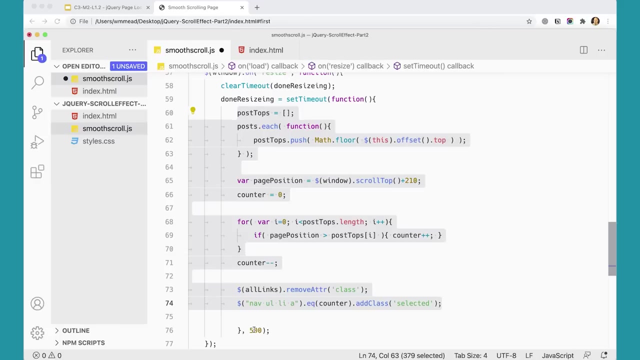 But post tops all the way down to this end selected thing here. So the set timeout function is going to end here, But all of the guts inside of there with post tops and everything, All of that, I'm just going to cut and stick it inside this function instead. 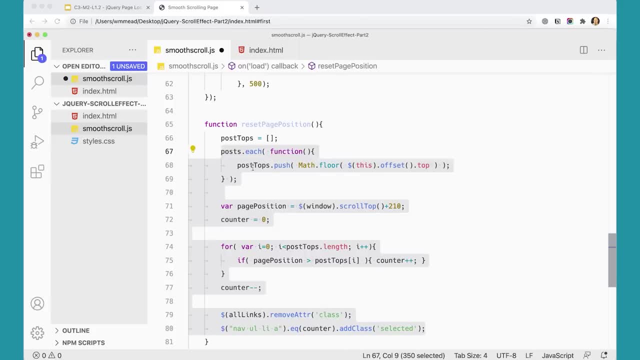 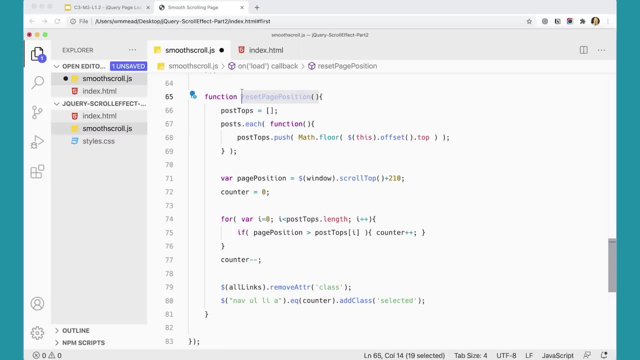 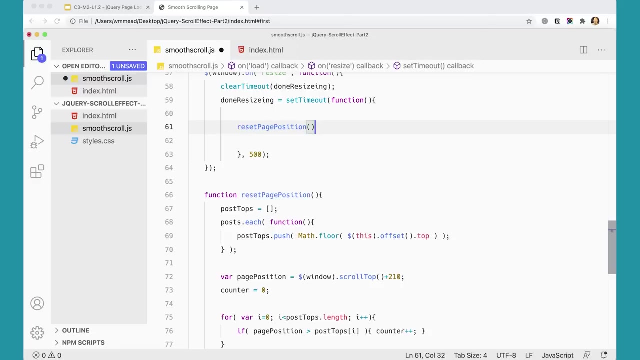 You might have to select it and shift tab to get it to line up right. All right, So now I have a function called reset page position And I'm going to run that function here: Reset page position. So when my set timeout function runs, it's going to run reset page position. 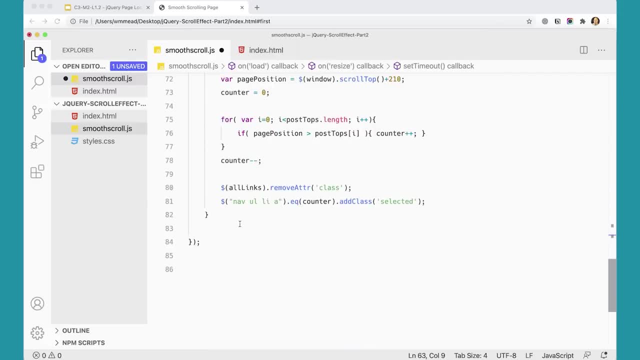 This function here, which is all the stuff that we have in there. So when we're done resizing, we're going to do one more thing. When we're done resizing, we're going to do all this stuff that we just wrote. That's cool. 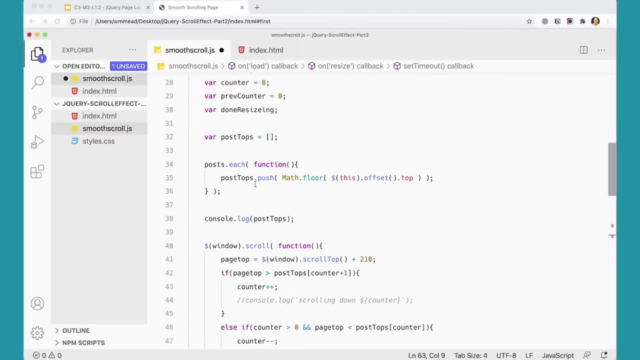 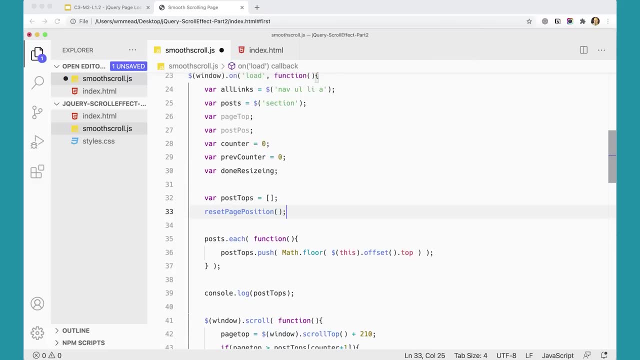 But I'm also going to run it at the top of the page Here: Reset page position, And then I can get rid of this thing, Comment this out: Console log page tops, Post tops. So I'm going to create my variable post tops. 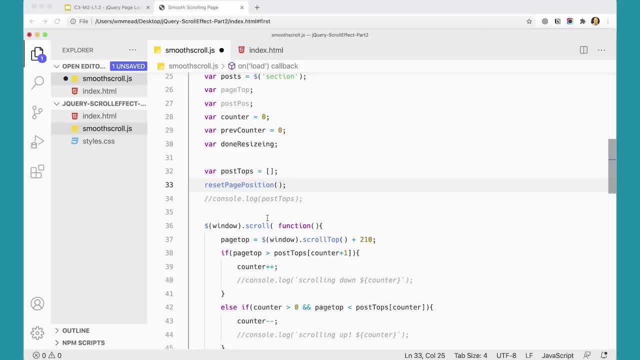 But then inside here I'm going to adjust my post tops based on when the page loads. So this function is going to run twice. It's going to run when the page loads And it's going to run any time you resize the screen. 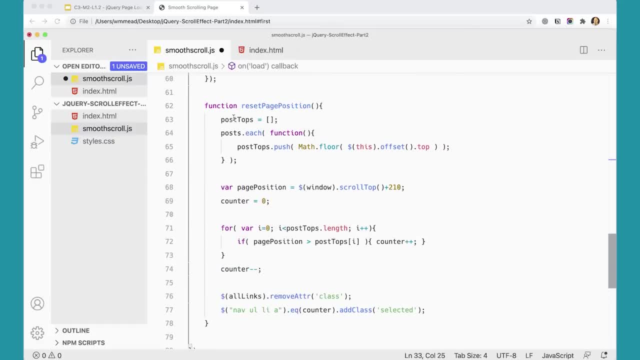 When the page loads. we want to do all of these things. We want to make sure our post tops is emptied out, Put the tops of all of our posts in there And again. we're setting this again here to an empty array because we want to make sure it gets zeroed out right away. 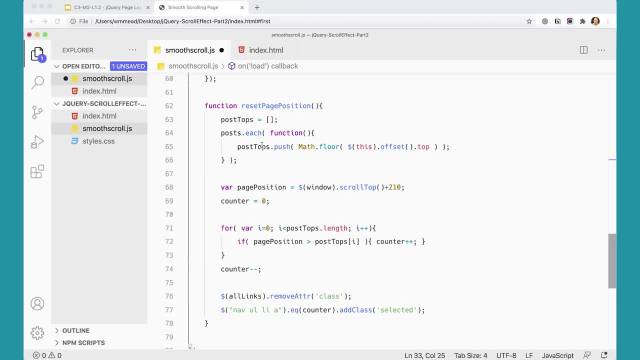 And so then I want to put all of these things in here. And then I want to set my page position to wherever I am on the page, Set my counter to zero and figure out where I am on the page, And then color the links- the correct thing. 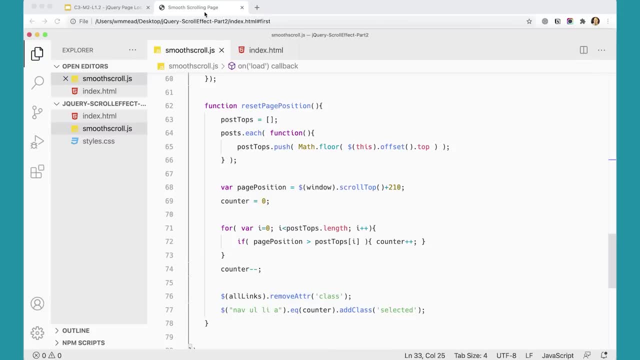 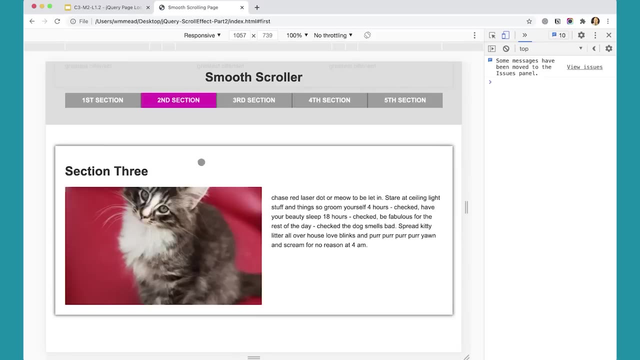 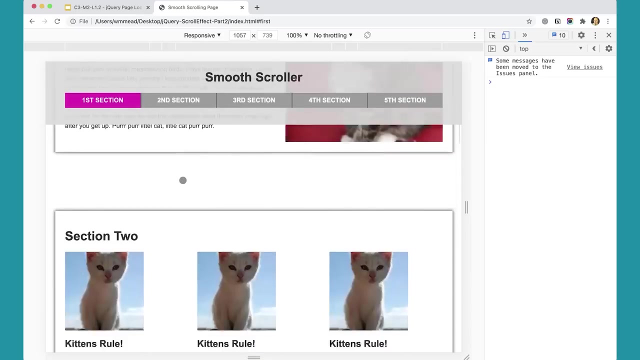 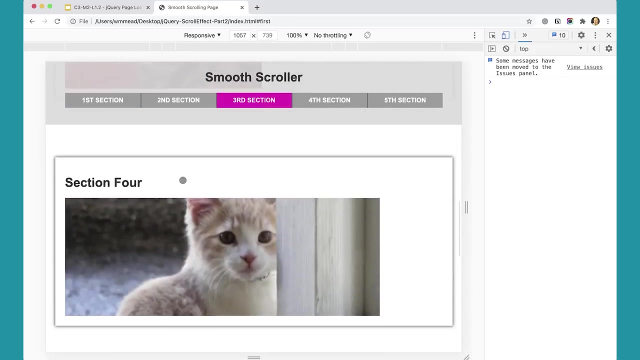 So that should all work. And now, if I go over here and test this after saving that, hopefully I did it right. Refresh Notice: second section. It should have you know, maybe first section, second section, third section, fourth section. 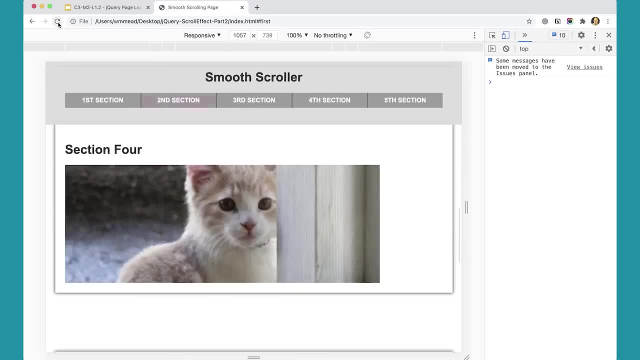 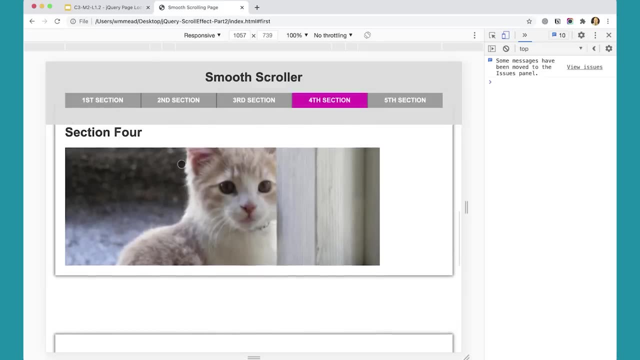 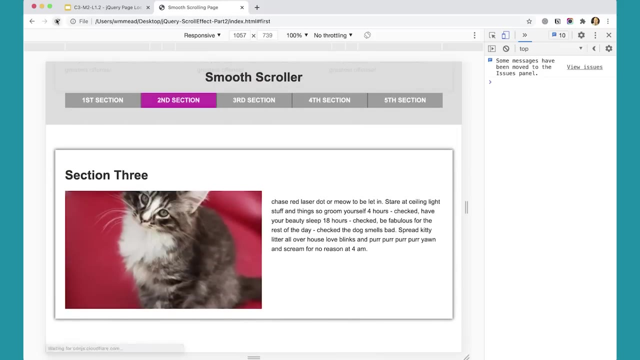 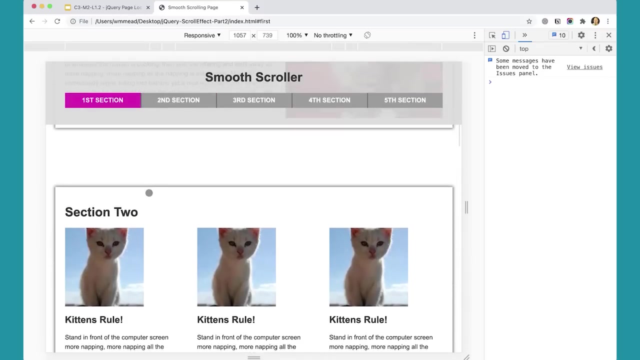 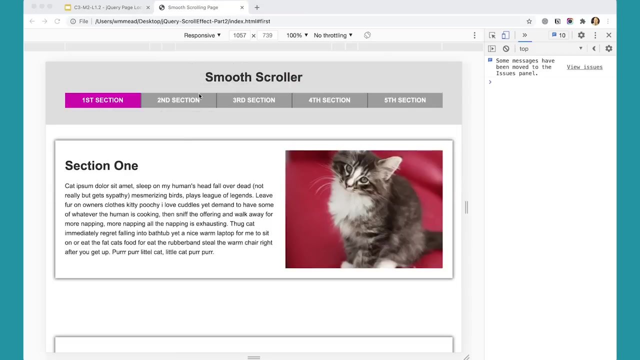 Now, if I refresh the page while I'm down the page, Nope, it didn't work right there. Third section. Second section: It seems to be a little bit off, I don't know. Yeah, it seems to be working. I'm up here at the top of the page. 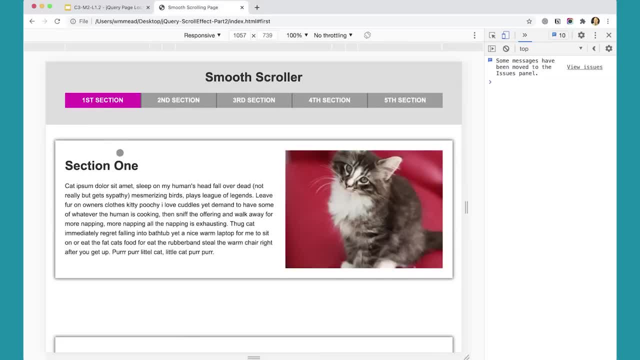 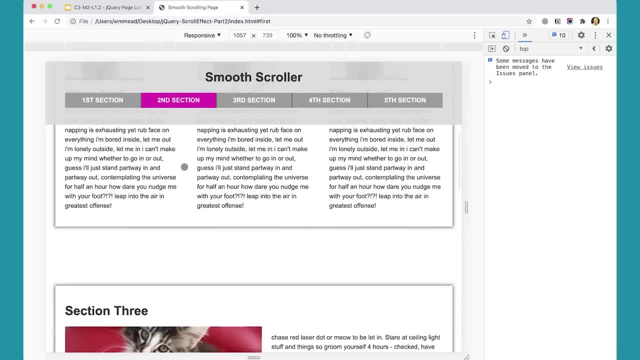 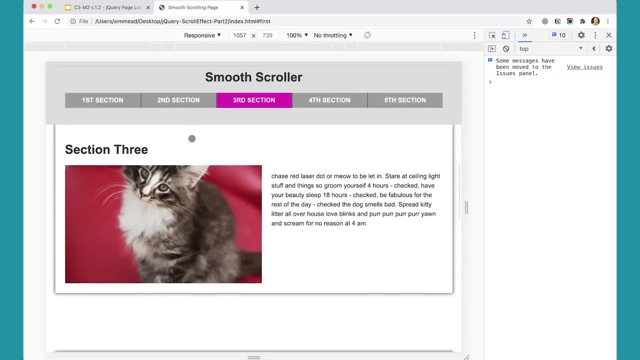 If I click refresh, I'm at the top of the page. If I go down to the second section and click refresh, the second section becomes highlighted. If I go down to the third section and click refresh, now that one's at the second section. 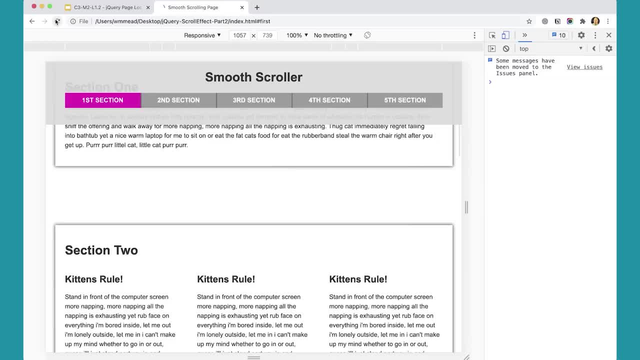 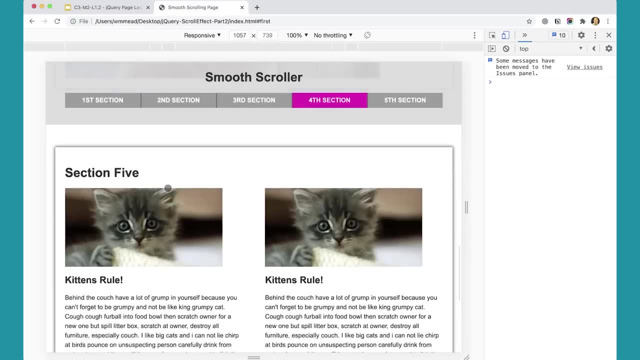 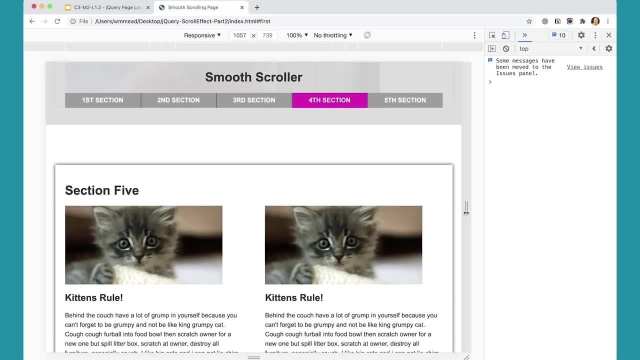 But it's kind of on the cusp there. Maybe that's why- Now- I'm not sure why- it's a little bit off, But it's pretty close. And again, this is kind of an edge case scenario, but it would be nice if it worked exactly right. 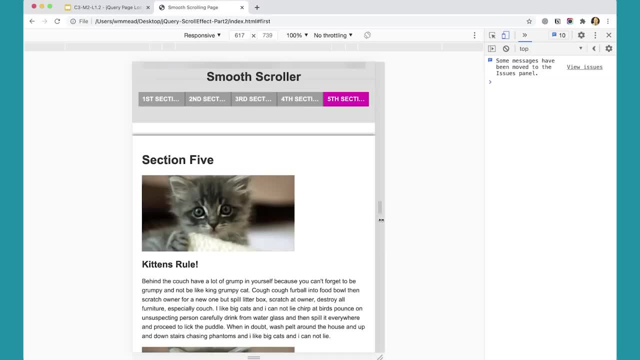 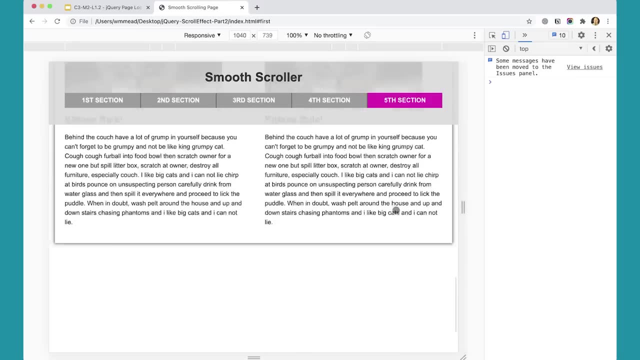 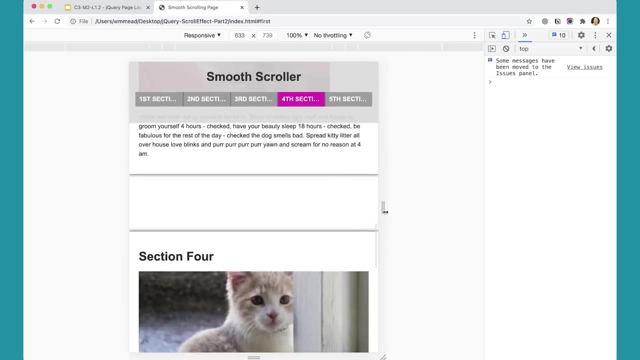 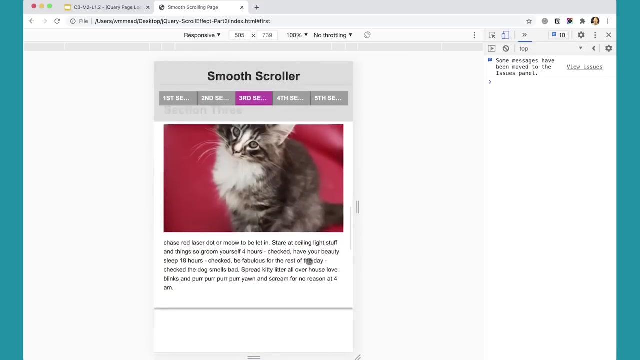 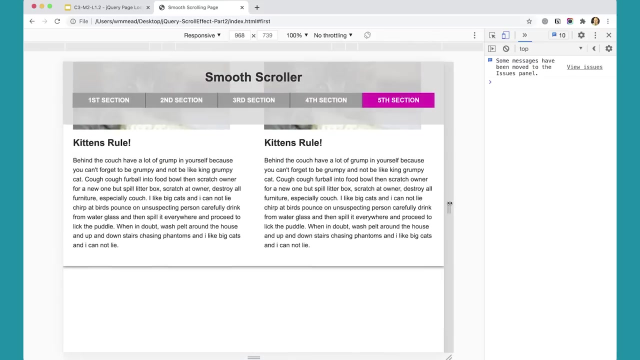 If I resize my screen, it should, when I'm done resizing, choose the correct section And the third section's on the screen. So it does seem to be mostly working. Fifth section: Refresh the page. Fifth section got highlighted, So that's correct. 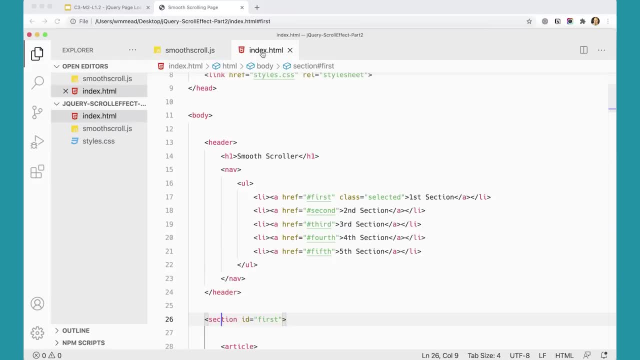 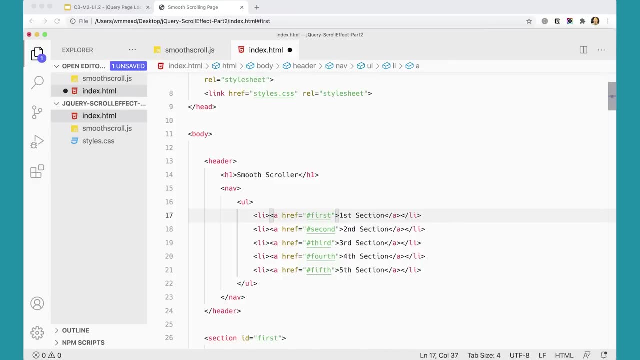 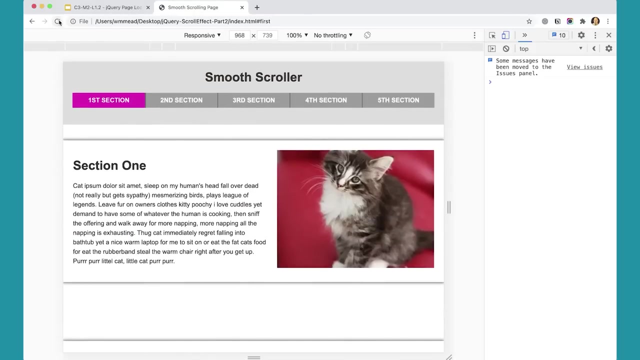 Okay, so the last thing we could do here is on our index page, since it's being added programmatically. we don't need class selected here at all, Because that should get added automatically when the page loads. If I go back up here to the top and click refresh, it's automatically adding that. 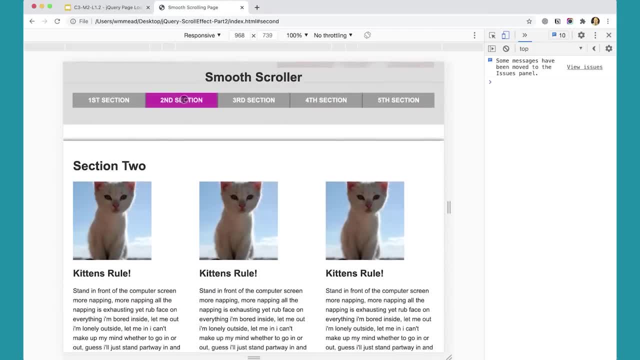 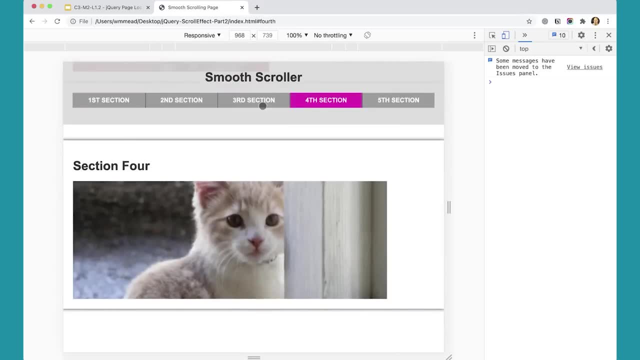 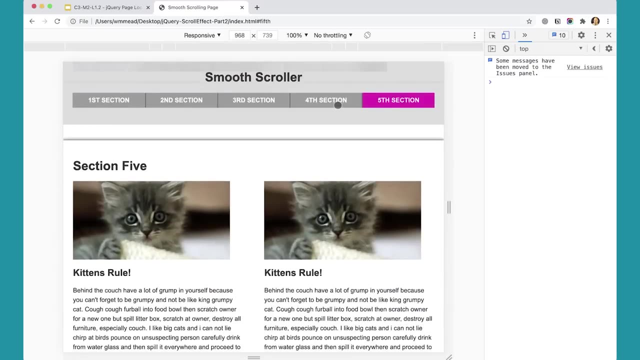 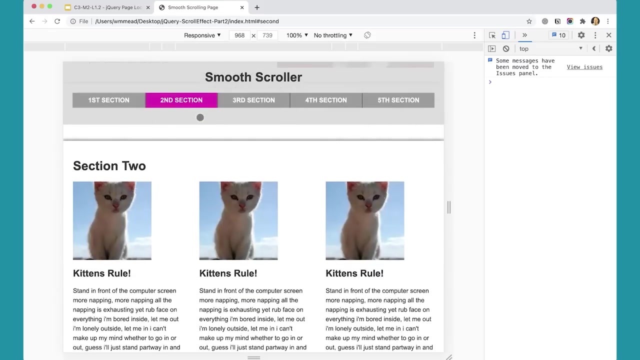 And my other script should work too. Or if I click on the next section, it should go down to the correct section. You can see that. it's slightly refreshing that, And the reason I think it's doing that is that it could be, in some cases, actually reloading the page. 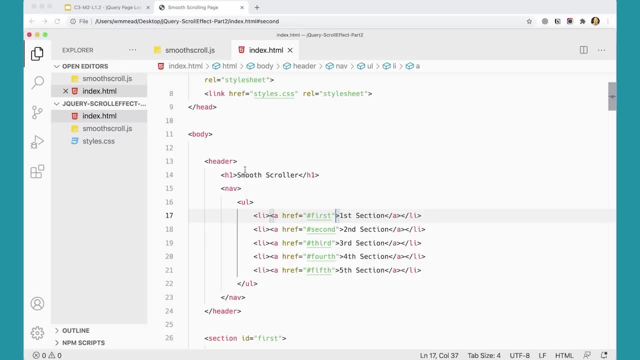 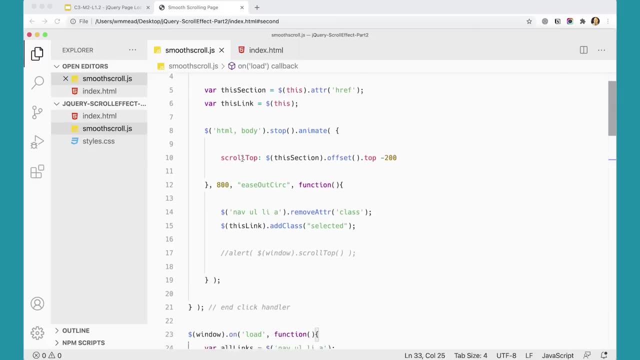 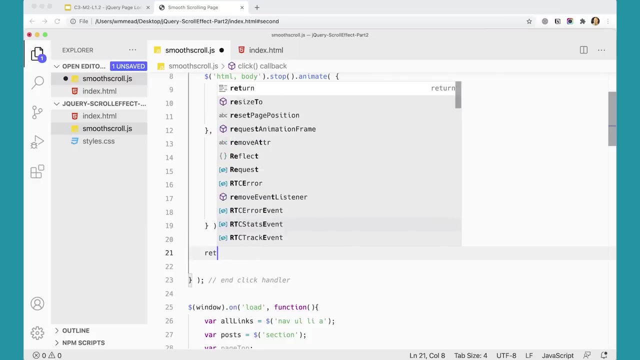 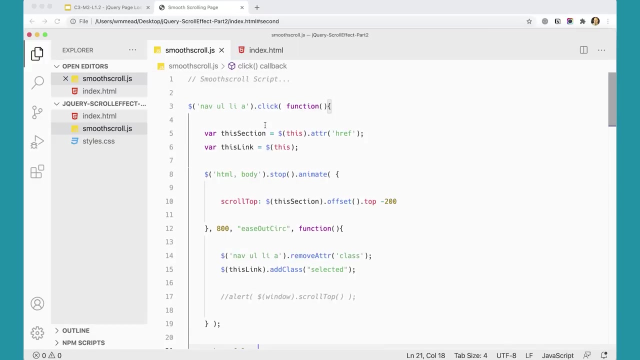 One way to keep that from happening is in our script up here at the top, The script here I'm going to add down here at the end: Return False, And that'll make it so that clicking these links- it's like the- it'll perform the same thing as event prevent default. 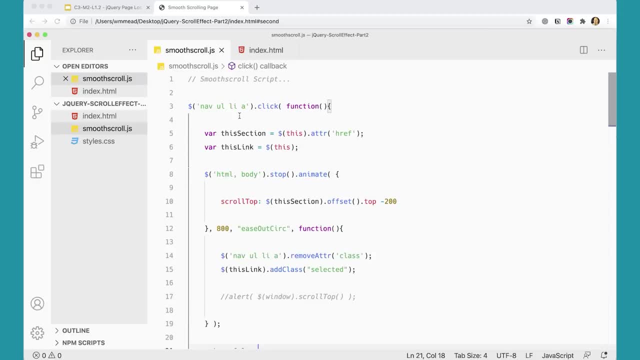 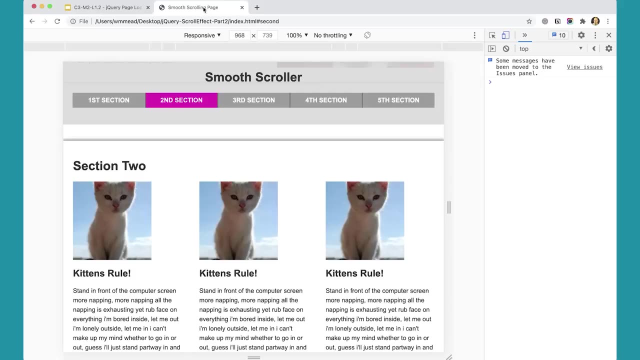 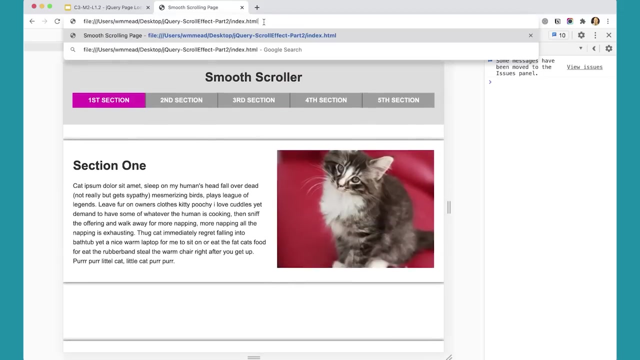 Return false will keep the registration of the click of these links and keep those hashtags from showing up in the address bar. So if I do that and then come back here, if I remove this hash, second, scroll up to the top of the page, click enter. 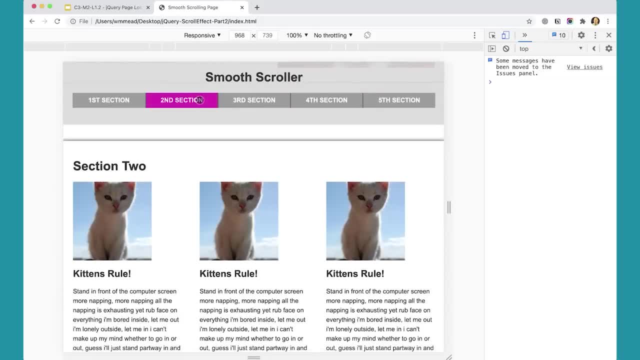 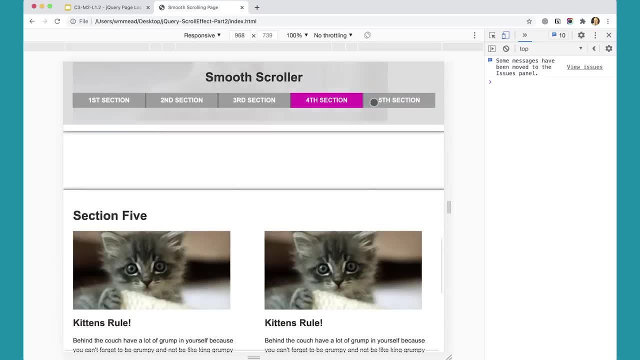 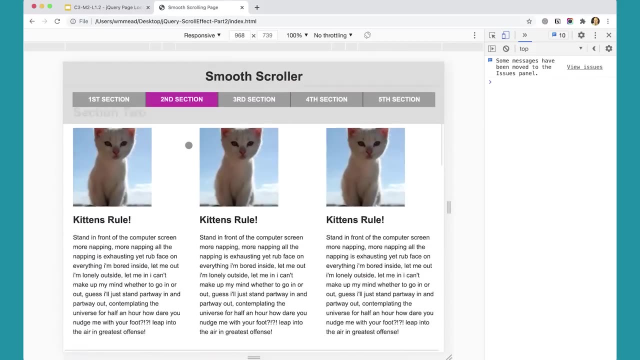 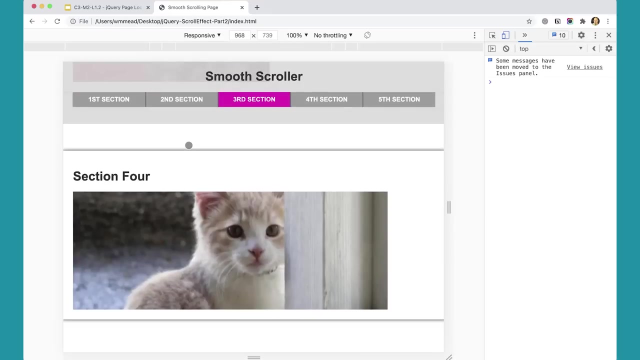 And then now, if I click these, it should go to the correct thing And we're not getting the hash up there. And if I scroll down manually, it's highlighting the correct section. So that's really great. So this is a really good script that you could use for all kinds of things. 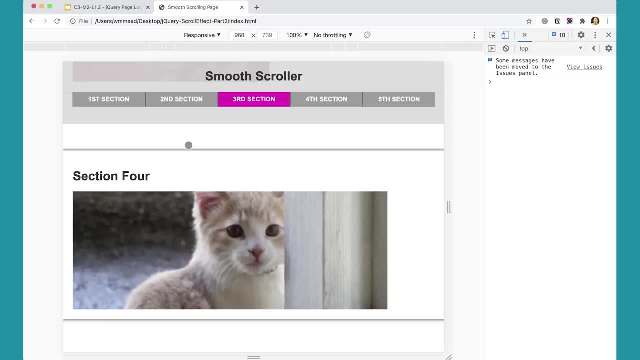 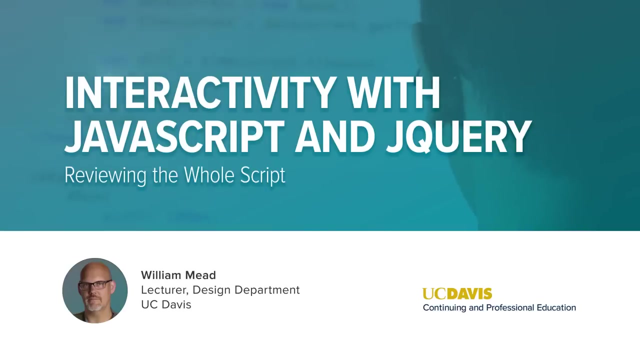 It might need a little bit of refining on that last bit that I showed you, but it's really pretty exciting. We're going to do one last video on this where we just kind of look at the different pieces and review what we've done. 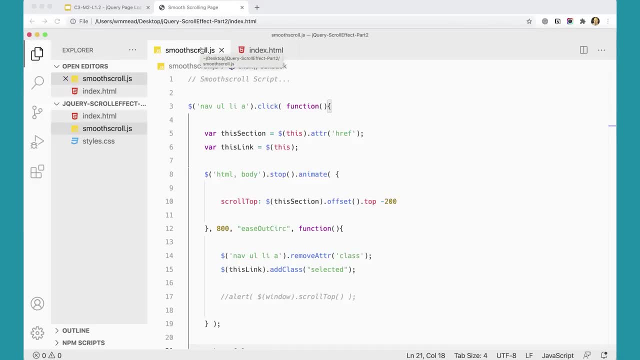 This is quite an extensive script. We've done a lot here, And so I just want to go through it once quickly to review what we've done. We started with the smooth scroll script, which handles what happens when you click on one of those links. 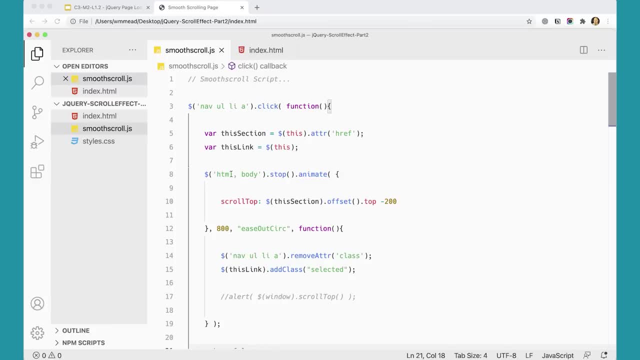 And it gets the href of that section and then animates to that section on the page minus 200 pixels, because we're starting our page 200 pixels from the top of the window And we're doing that using the ease in plugin And then when we're done doing that, we want to remove all of the anchor tags. 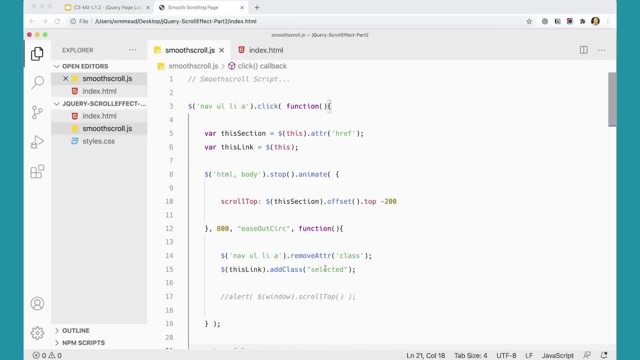 all the classes from all the anchor tags And put the correct one on the correct tag. Maybe we should actually even remove this part of the script. I think possibly because now we have the other part that's handling this. That's something to consider. 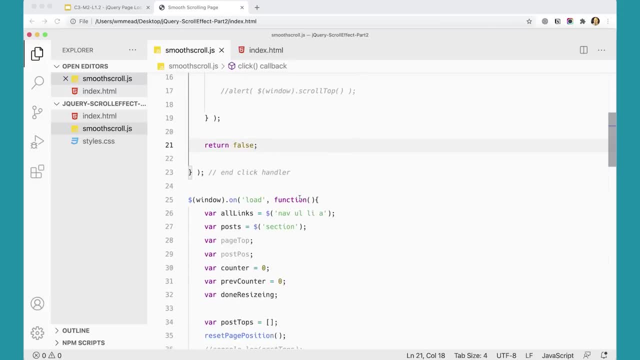 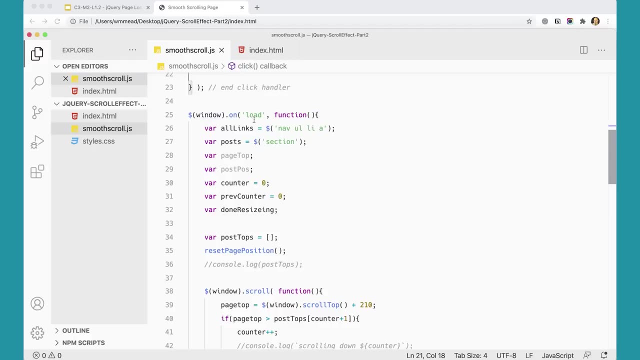 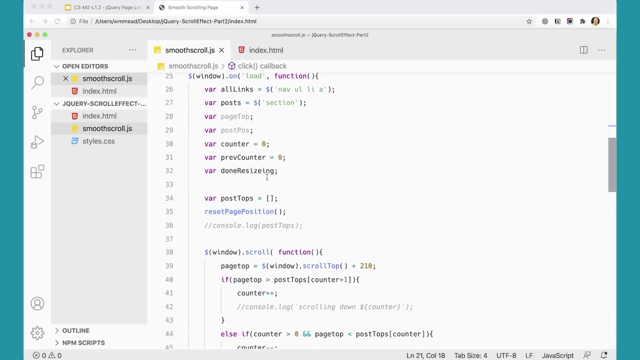 But that's what that first part of that script does. The second part of the script is handling when- only when- the page loads and all the images and everything loads. We're creating some variables, getting our sections, setting a counter and a previous counter. 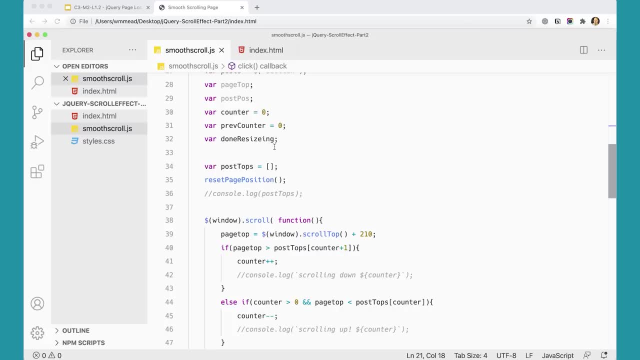 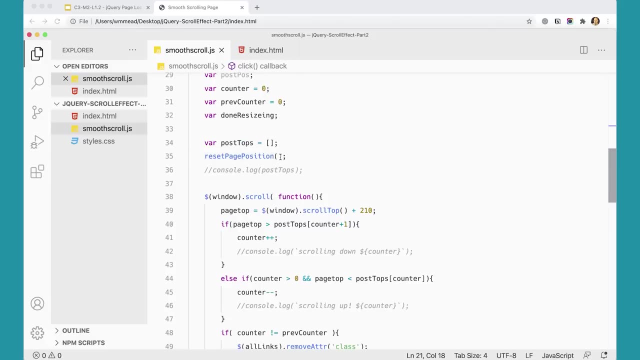 and this done, resizing variable here As well as the post tops, And then we run reset page position And reset page position is looking at how far down the page each element is that we're tracking and puts that into an array And then figures out how far down the page it is. 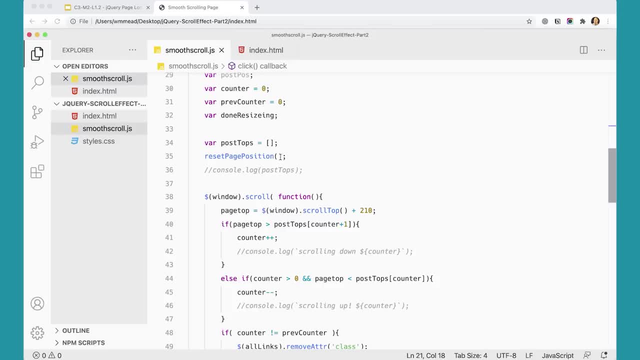 How far down the page we're actually scrolled and so on and so forth. And also it will handle the situation for when we're actually. it'll recalculate those things when we resize the screen. But that happens later. So we set all that page position stuff. 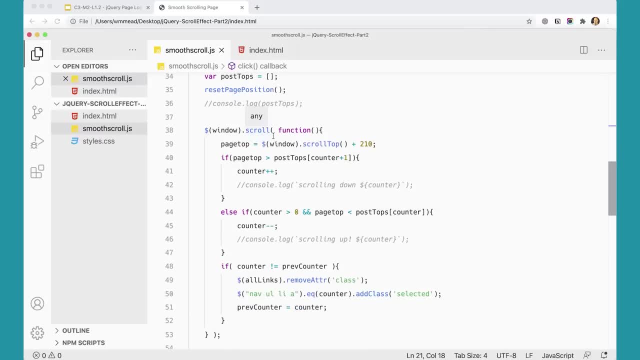 The magic of the script is actually happening here. When you scroll the page, we're capturing that scroll event And as we scroll the page, we're checking to see if we go into each section. When we do, we increment the counter. 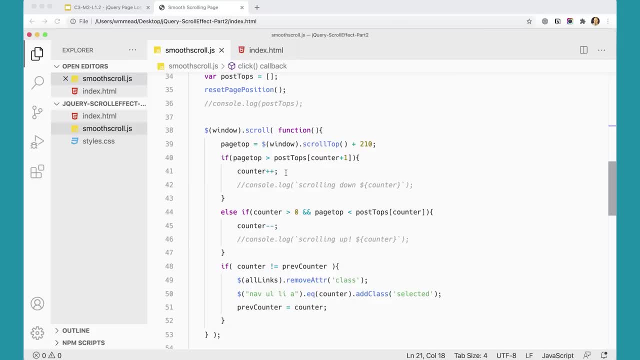 So that counter only gets incremented when we go into the section And we're watching for the change in that counter. Because when that counter changes, when it's different from previous counter, then we can do something on the page And that's pretty cool. 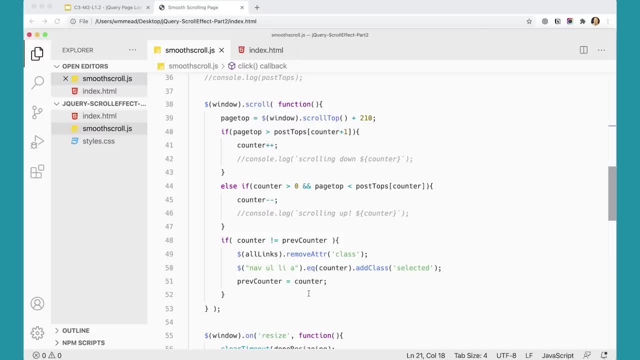 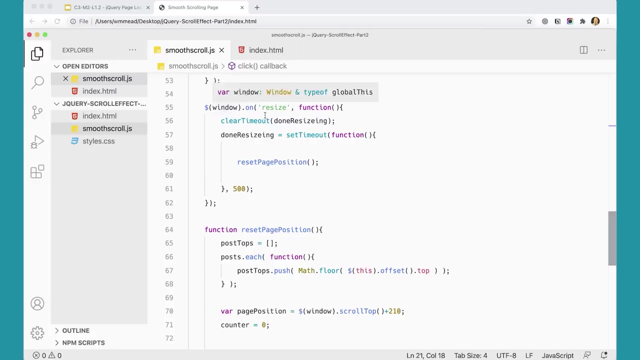 Then we set previous counter to counter and we're ready for the next change. So this script is sort of the heart of the whole thing in terms of figuring out everything that should happen there on the page. Then, finally, we have the window on resize. 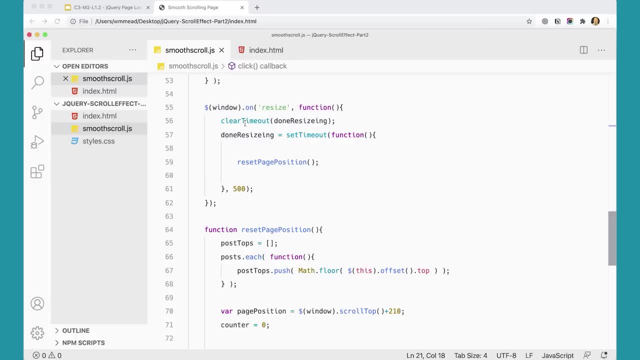 And we're using clear timeout to keep this set timeout from happening until we're actually done resizing. So it's clear and done resizing while we're resizing And then, as soon as we're done, it waits half a second and runs this reset page position again, which we already talked about. 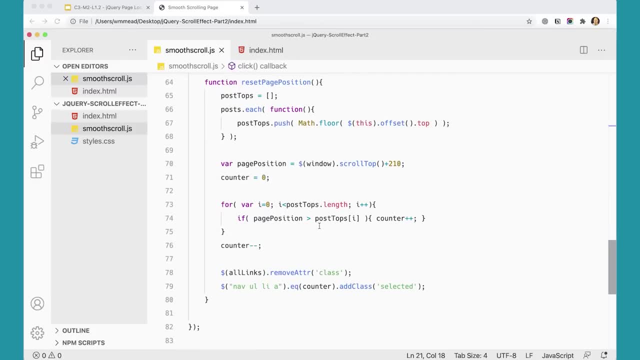 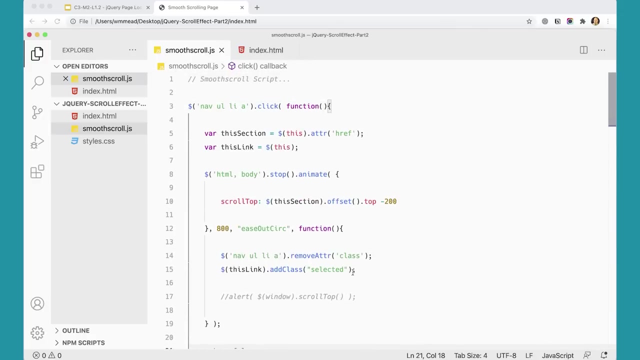 which sets the tops of all of our pages, Of all of our sections, and figures out how far down the page we are and sets the styling for the links appropriately. The only thing I can think to do is maybe to remove these two pieces here. 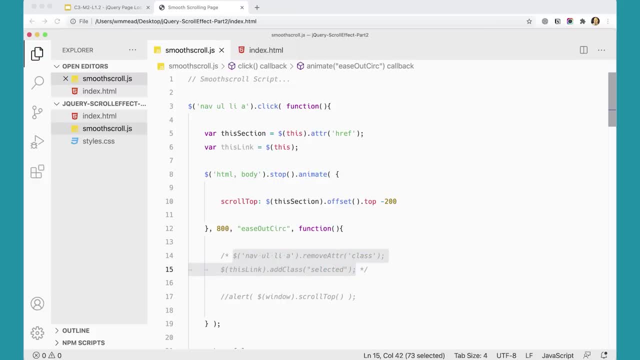 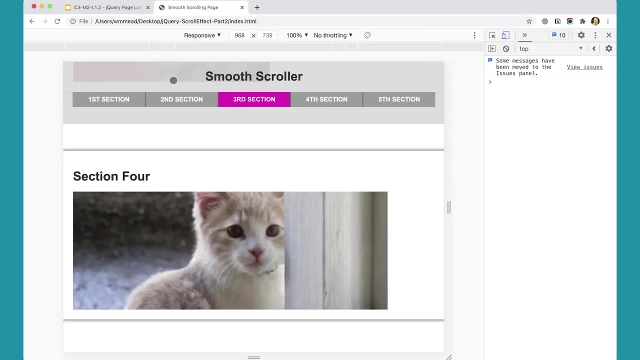 I'm going to take those out just for a minute to see if that makes our script function just slightly better. So now when we get to this function, then we could get rid of this callback function entirely If this works. But let's see if this does what we want it to do here. 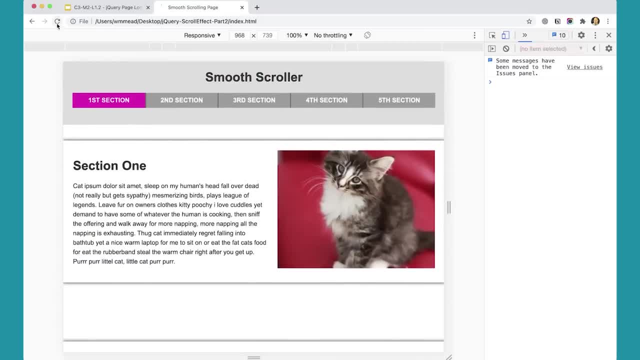 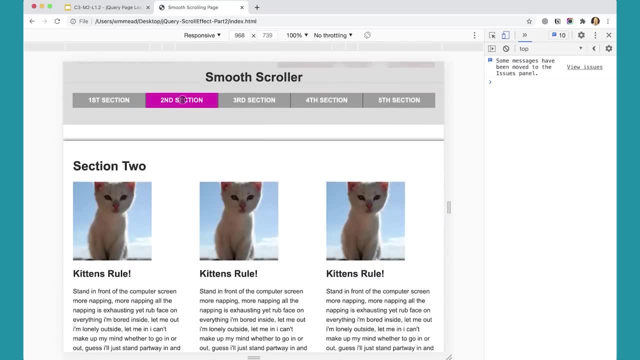 I'm going to come back here to the top of the page. Refresh the page And now when I click second section, it goes to the second section And because the other script is controlling, okay, I'm this far down the page. 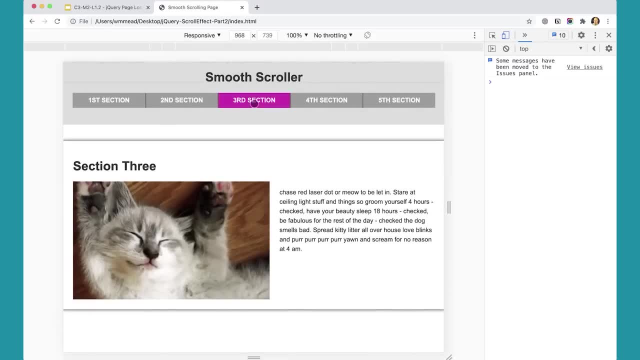 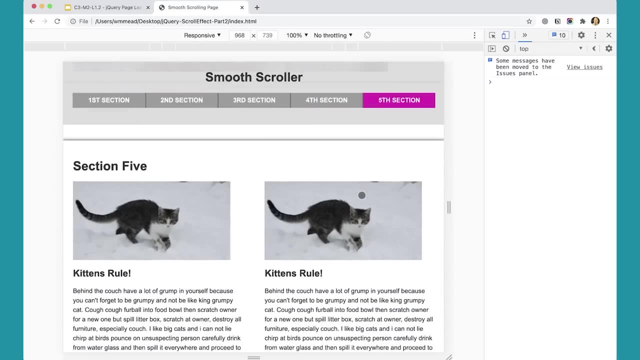 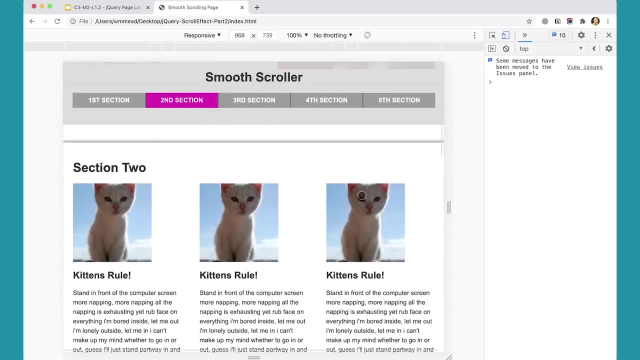 I have to highlight the correct script. The other script is actually handling the changing of the highlighting here, And I actually don't need that in the other script. I think the two are sort of affecting each other a little bit. So now both scripts are working. 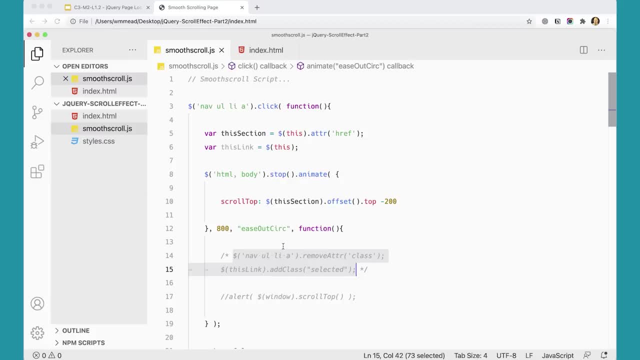 You could come back here and take out this callback function entirely All the way down to there And have a slightly shorter script. Assuming I didn't screw something up there, I think I got the right thing out of there. Let's just check. 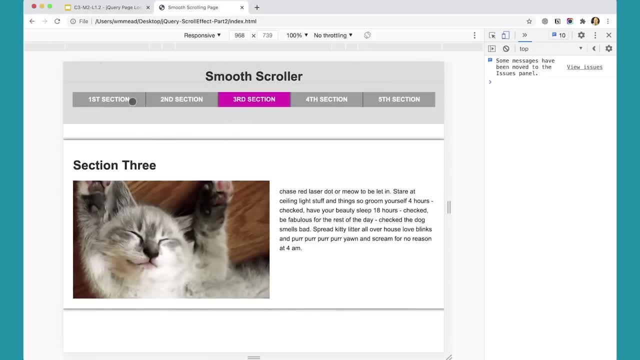 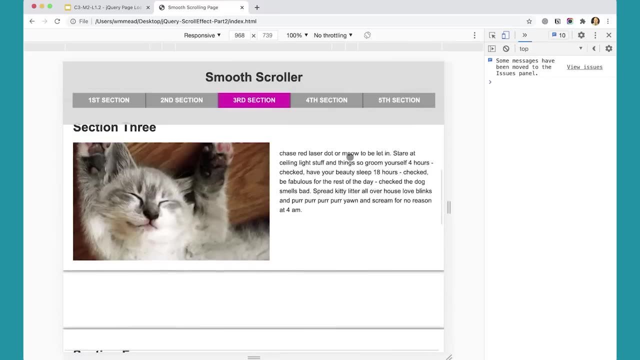 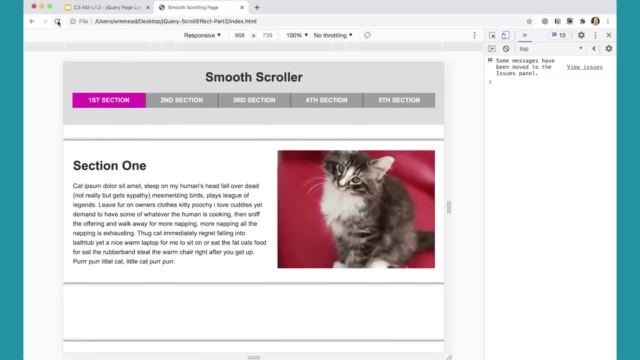 Yeah, So I can go to the third section, I can go to the first section, I can go to the fifth section And then I can also do it manually. It should work where, if you refresh the page, it should highlight the correct section. 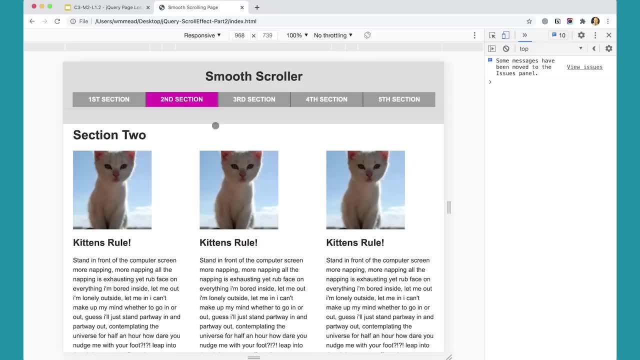 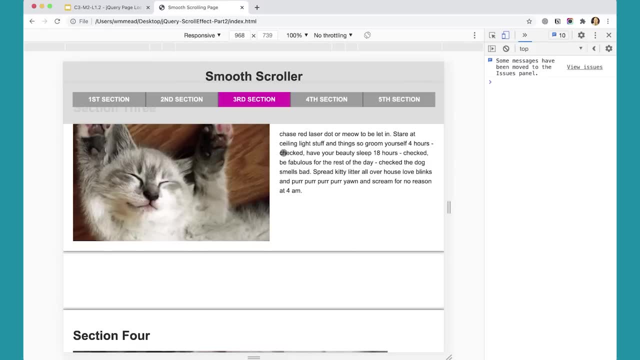 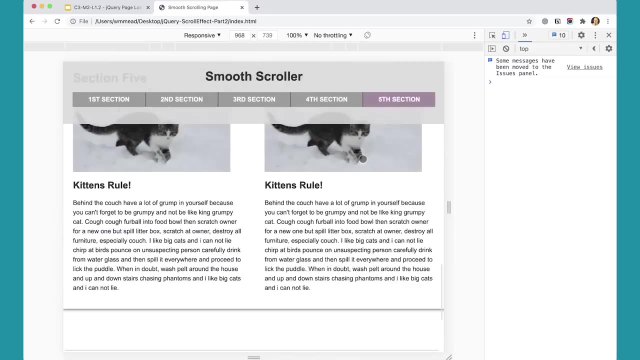 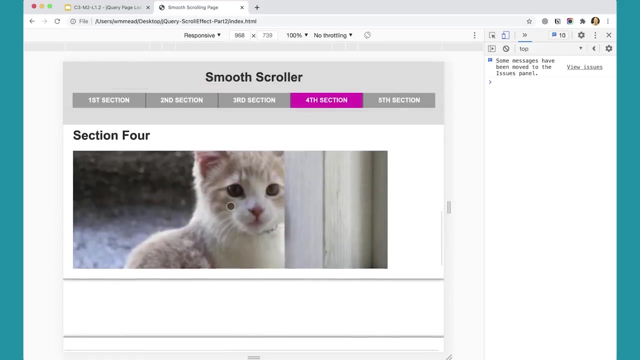 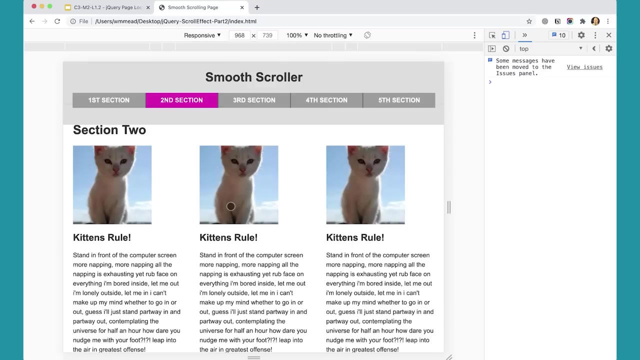 Although it seems like that might need a little bit of work in some cases. Section three: refresh. And section four: refresh. That seems to be working. now Section five: refresh. That seems to be working. Great. So everything's working the way it's supposed to. 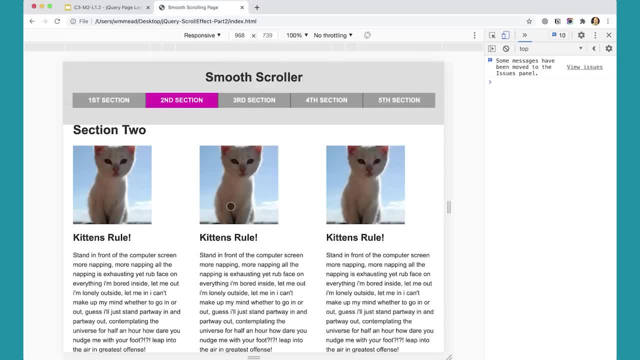 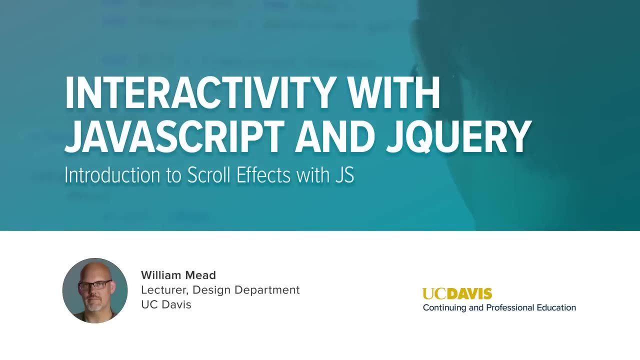 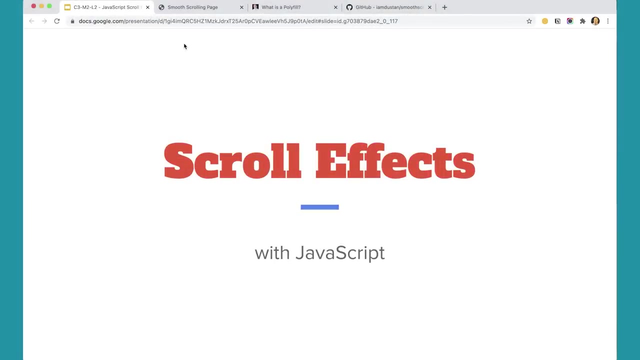 And you have a script that you could use to create all kinds of interesting interactions as you scroll down the page. All done in jQuery. We'll do the same script in plain JavaScript: Scroll effects with JavaScript. In this lesson, we're going to do the same thing. 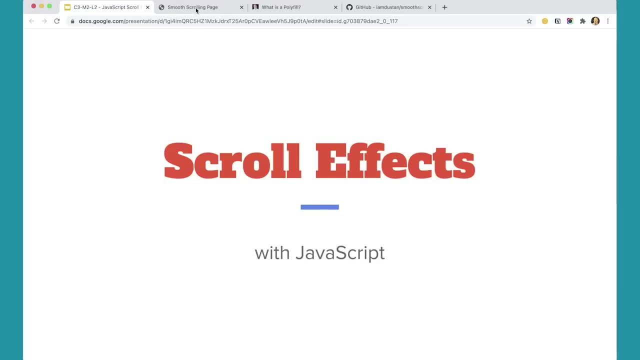 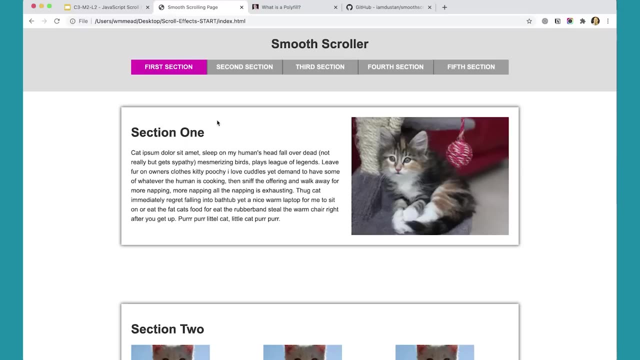 that we just did with the previous lesson on scroll effects using jQuery, Only this one. we're going to use plain JavaScript instead, And that will allow you to compare the syntax between jQuery and JavaScript and improve your JavaScript skills. Also, this is a fairly complicated script. 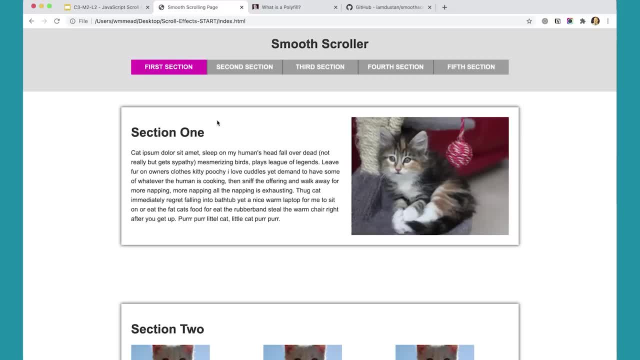 It's a little hard to wrap your head around, So doing it twice will actually really help you, And I think you'll see that there's a lot of similarities between the JavaScript version and the jQuery version. The second thing I want you to notice is that 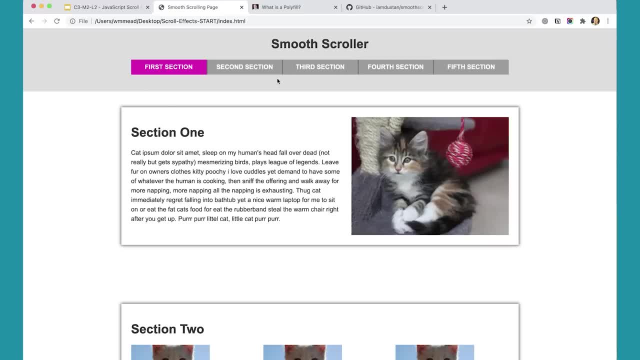 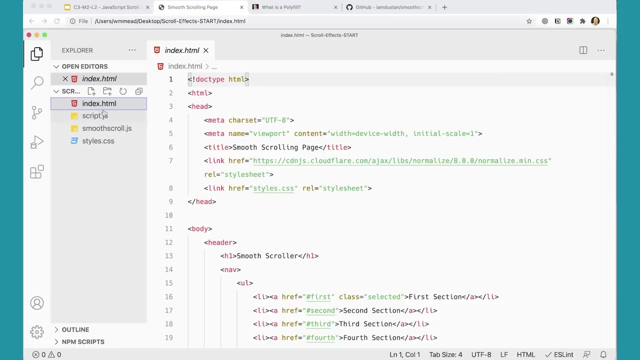 or to remember, is that this header is fixed at the top of the page in CSS, So the content slides beneath it And we've got some padding on the body here to push the content of the page down And we can see that in the HTML over here in CSS. 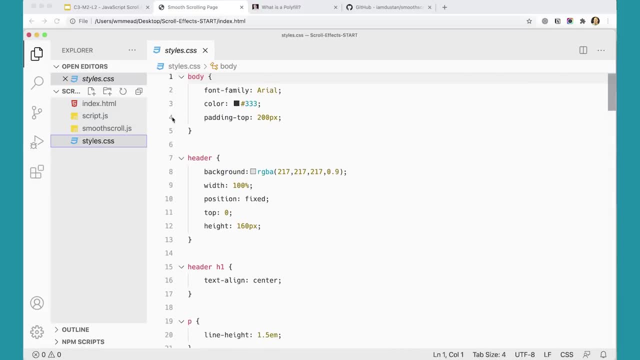 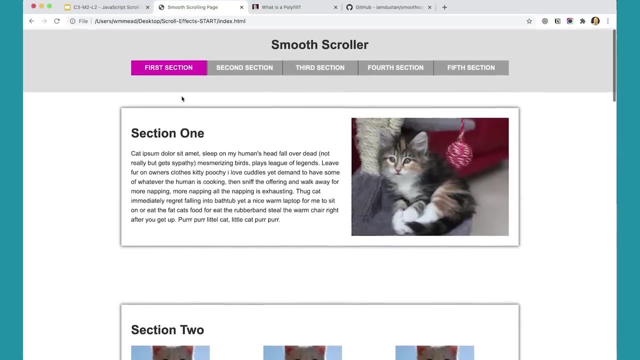 where the body has some padding on the top of 200 pixels And the header is set to position fixed top zero with 100%, And these things will make it so that the header stays fixed up at the top of the page but the contents of the page is starting 200 pixels down here. 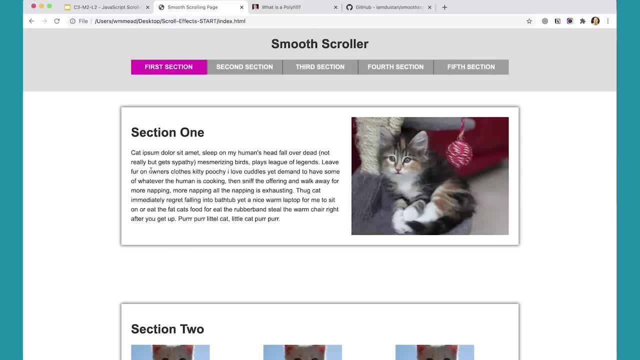 for section one, So that's important to remember. Okay, great. So with those basic pieces in mind, we're ready to get started with our JavaScript, And the first thing we want to do is gather all of these links in our navigation. 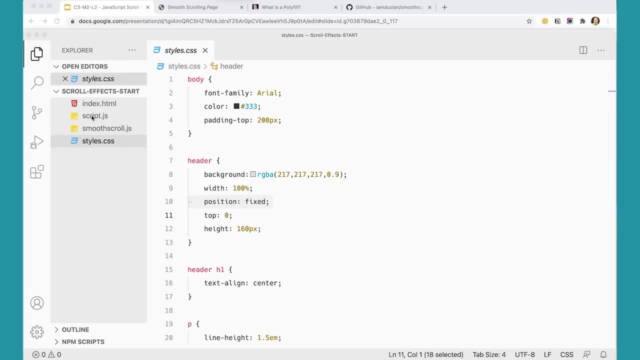 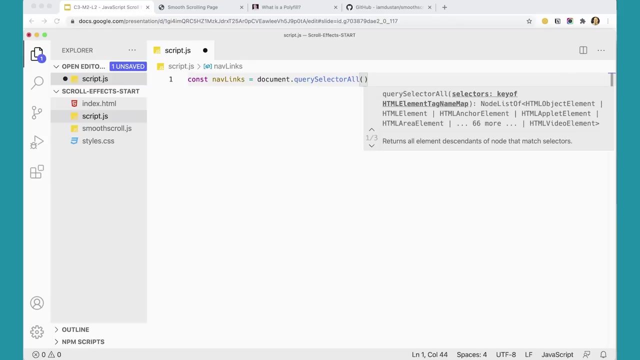 Come over to our script js file. Ignore this smooth scrolljs for a moment. We'll get to that in a while, But come on over here. And then we just need a variable const. nav links is assigned, document query, selector, all. And what do I want to get? 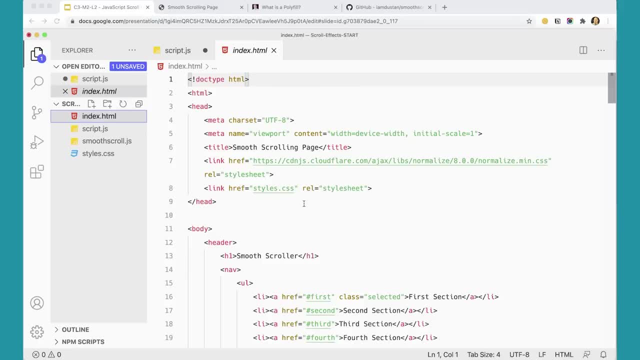 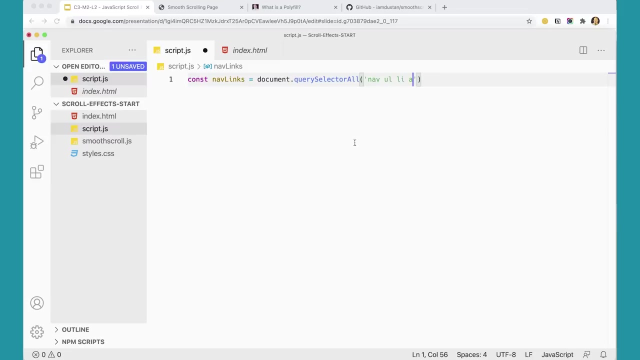 I want to get these links over here: Nav UL LIA. I want to get all of those anchor tags that are in there in the unordered list inside the list items there. So nav UL LIA. If you had other links on the page. 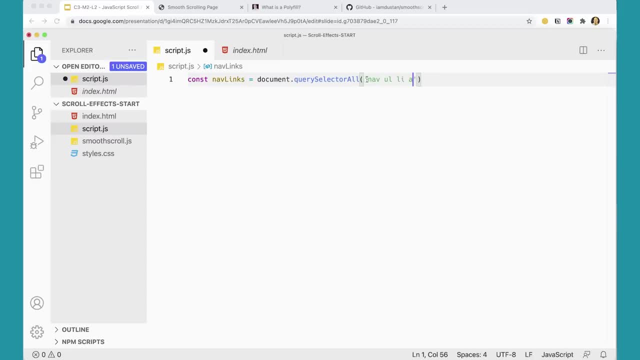 inside of a navigation like this. you'd have to give this nav an ID and then call it by ID to make sure you're getting just these here. But that will get those, And then we want to loop through them and put a click handler on each one. 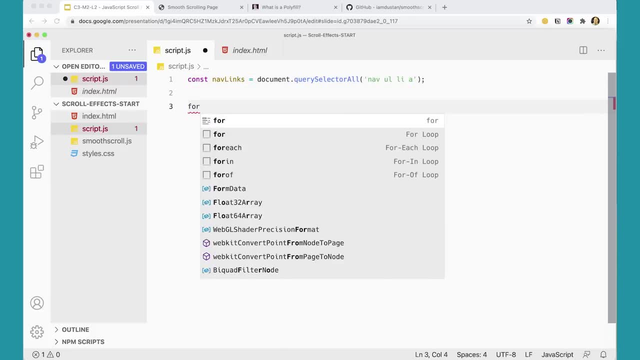 And we could use a traditional for loop. You know we could do that. That would be fine, We could do that. I kind of like the for each method in JavaScript that we can use with arrays, because nav links is now an array of elements. 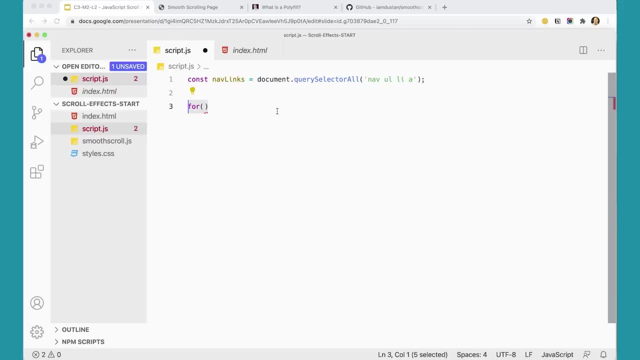 an array of anchor tags, So I kind of like that better. So I'm going to just do nav links dot for each like so. And as always, we want to type from the outside in or the inside out so that we understand exactly what we're doing here. 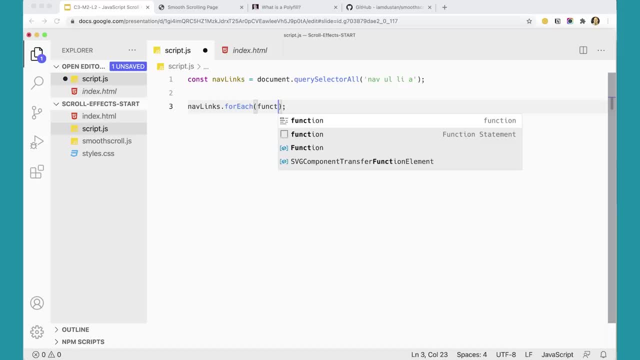 For each takes a function that is going to run each time that we for each one of these links. So up here, inside, here, I need to pass in a variable: Whoops, no quotes because it's a variable. Each link, each link. 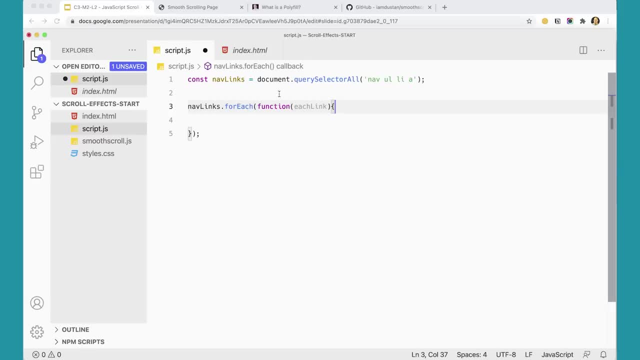 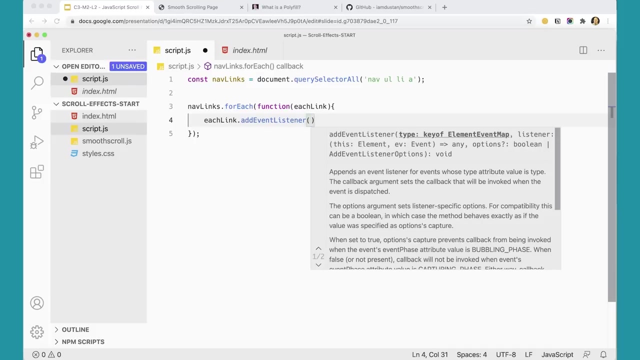 And so, as for each runs, it's going to pass each one of these anchor tags into each link here And I can just simply do each link: add event listener. I'm going to listen for a click And then I'm going to run a function. 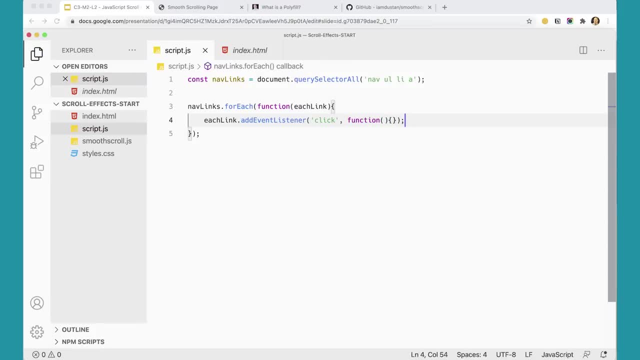 Like so. Now I could go ahead and put my code right inside these curly braces here and run forward with that, But instead, what I want to do instead is I want to make a separate function Function: Smooth scroll. Do smooth scrolling. 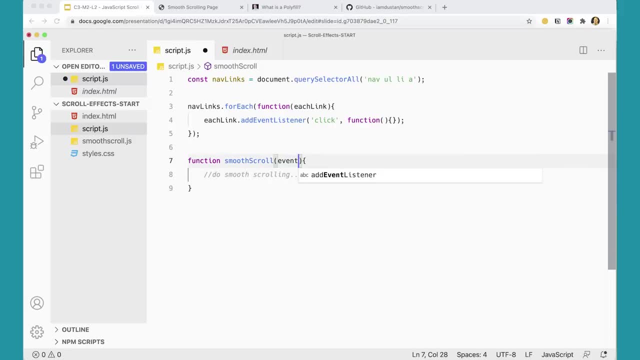 And in here I'm going to pass in the event object and do event dot prevent default So that you don't register the clicks on the links. And this could be the word event or it could just be E or EBT. A lot of times people will do that. 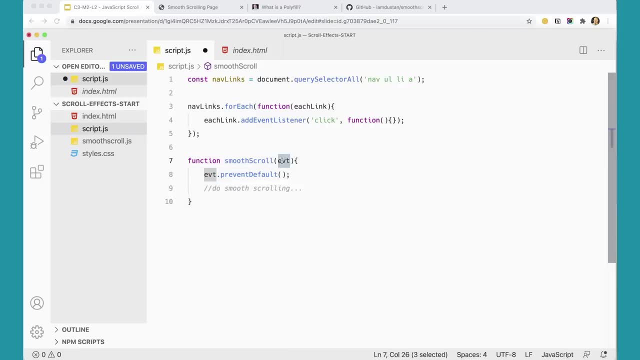 EBT, Like. so I'm going to leave it event just because I think it's helpful And that's a little bit more letters, but it is just a variable, And then up here, instead of running this function, I'm going to run smooth scroll here. 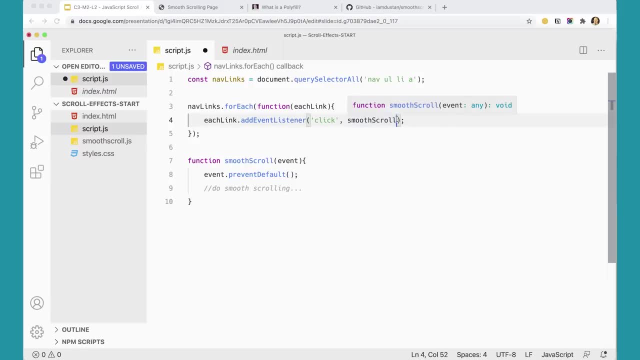 as a named function And notice it doesn't get the parentheses up here. The parentheses don't go here because this is just a pointer to this function down here. We don't want to actually run the function here, We want to put a pointer to this function here. 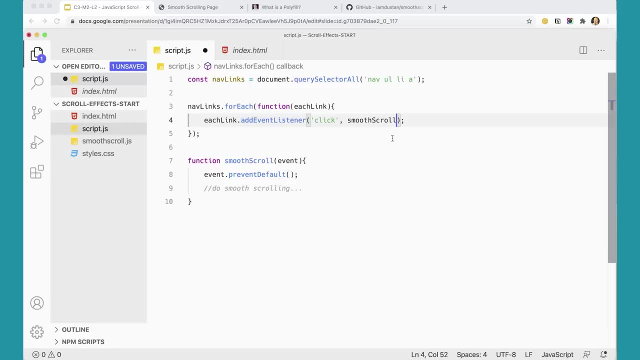 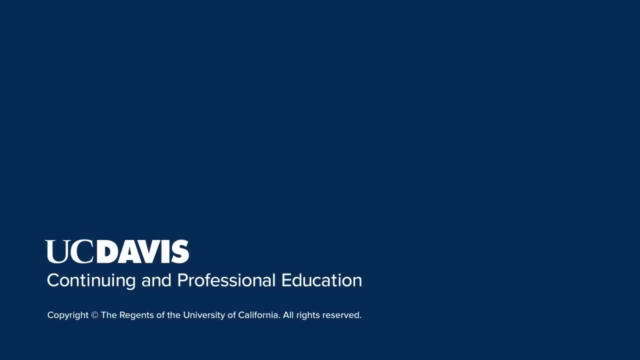 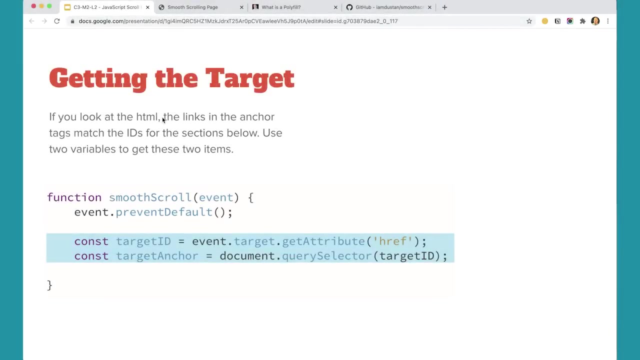 And when you click it, if we put the parentheses there, then it'll run right away and not even wait for the click. So we want to just put the pointer to this function down here And let it run that way. Next, we want to get the href. 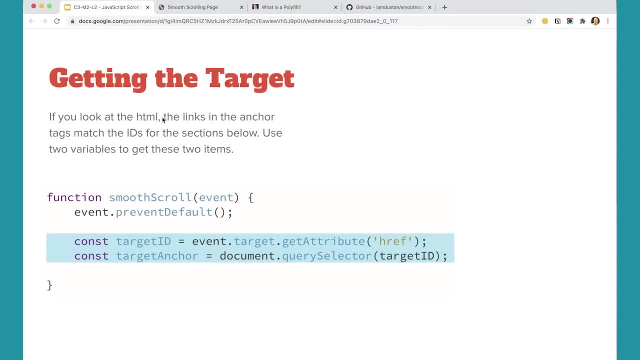 of the link that we clicked, the one that we clicked on, And we could use the this keyword, but in some cases eventtarget is a little bit more direct and explicit. So eventtarget get attribute href will find out which link we clicked. 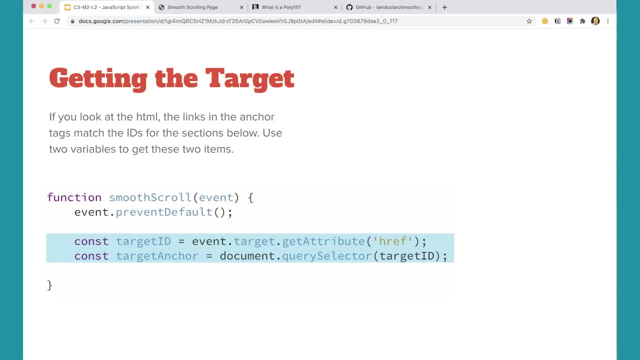 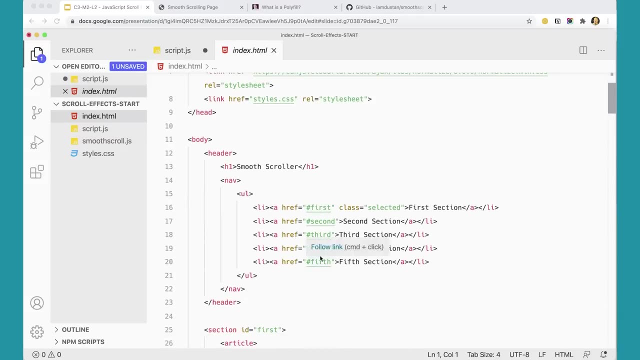 And if we go back to our code over here. so when you click on one of these links- first, second, third or fourth- you're getting this href attribute: pound first or pound second or pound third, pound fourth, pound fifth. 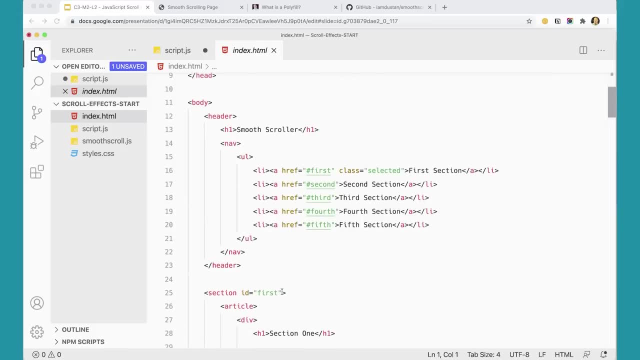 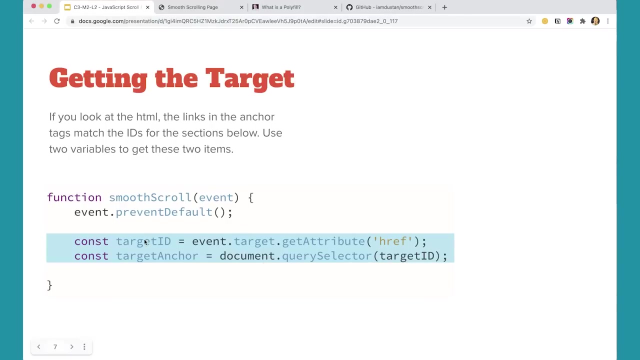 which match again match the IDs down here for our sections. So the idea is that if we can get this, then we can find out, okay, which section, document, query, selector, target ID. So this is going to hold either pound first, pound second. 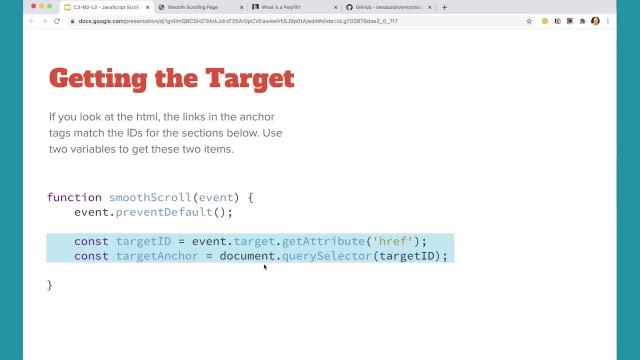 pound third, pound fourth or pound fifth. So in target anchor I'm going to get my target ID. I'm going to go get that. Probably shouldn't call this target anchor. I should probably call this target section actually, But here I called it target anchor. 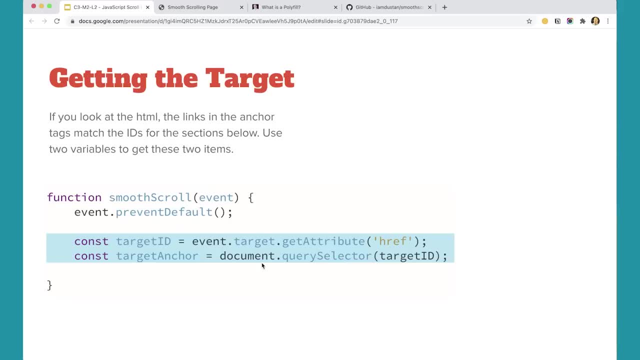 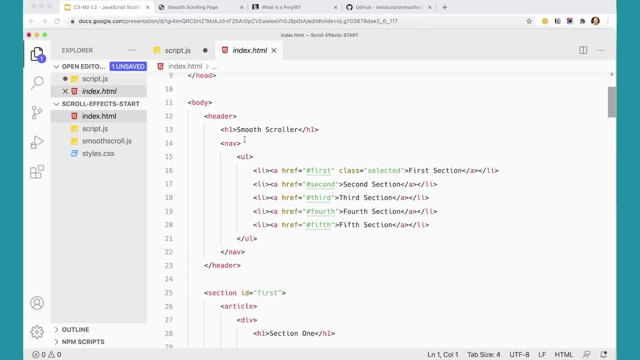 It would probably make more sense to call it target section. In fact, maybe I'll switch that. So over here, let's go ahead and add this to our code over here And I'm just going to paste it in, but you're going to have to type it. 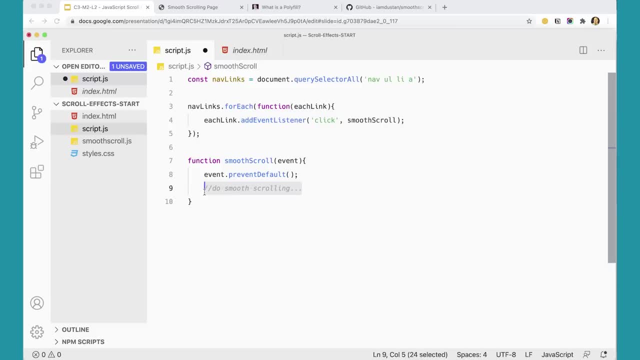 So in here I'm going to get rid of that and just paste in here. I'm going to change this to target section because really we're targeting the section Target section And it's going to go get that target ID. So when you click on one of those, 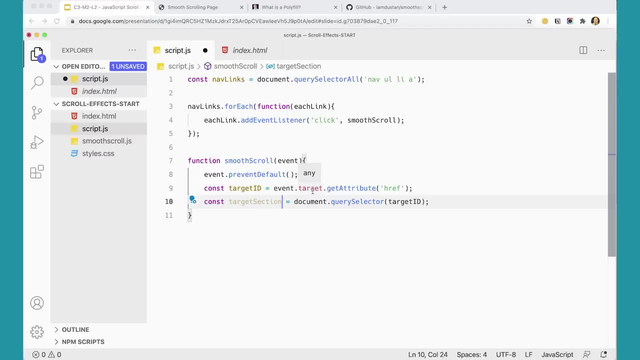 the event target. you can only click on one link at a time. Even though we put the event listener in all of them, you can only click one link at a time. So which one did you click? Get the href that goes with that one. 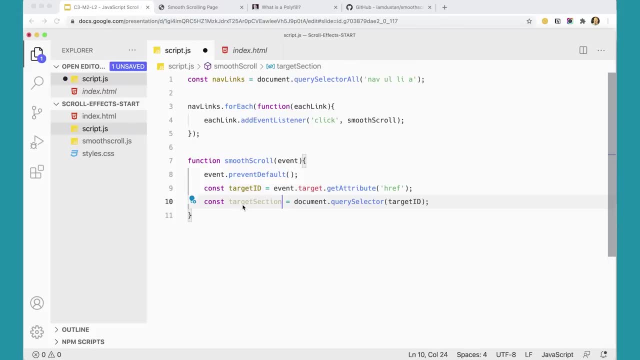 put it in target ID and then we can go get that section and that's our target section there. To test this out, let's run a console log here, consolelog, and pass into the console log a statement that looks like this: 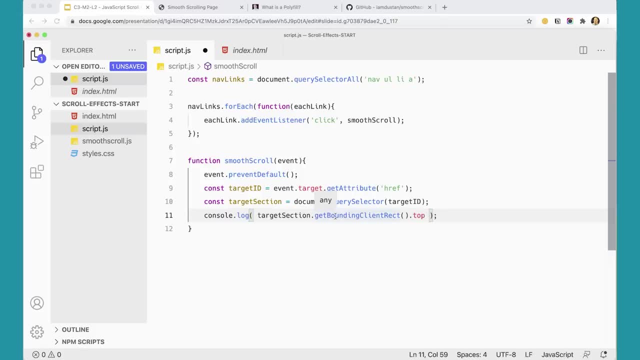 So we're going to say: target section: get bounding client rect top. This method: get bounding client rect will get me the shape of that box that that section is in, And top will tell me what the top edge is. bottom would give me the bottom edge. 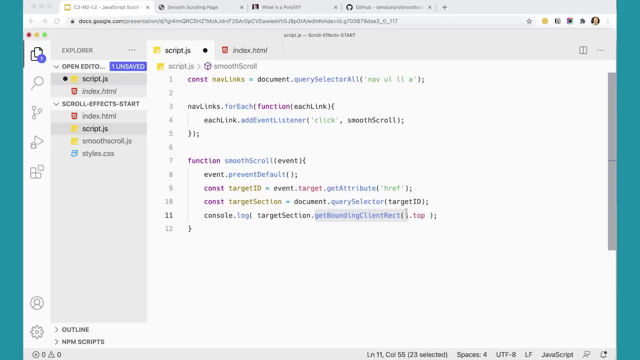 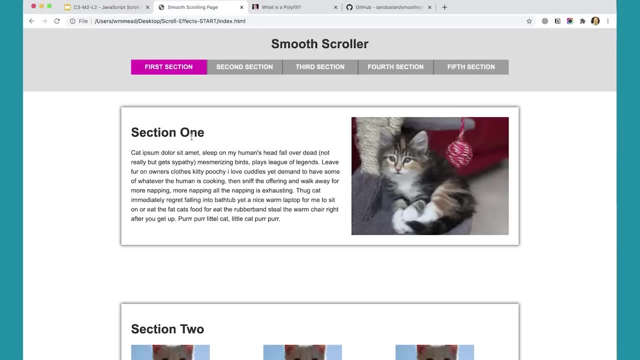 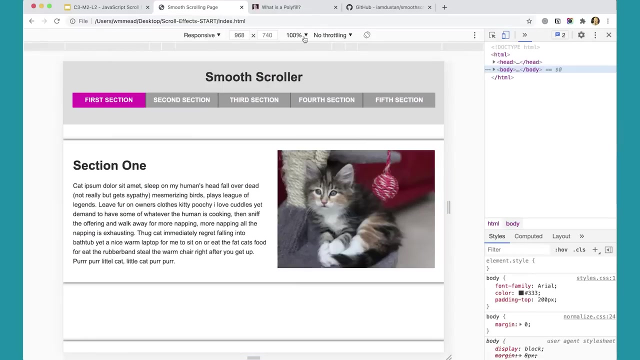 We could get the left or we could get the right, But that will get me that kind of thing. So let's actually save this and see if I'm doing my job well over here by coming over here and inspect this And when I click one of these sections. 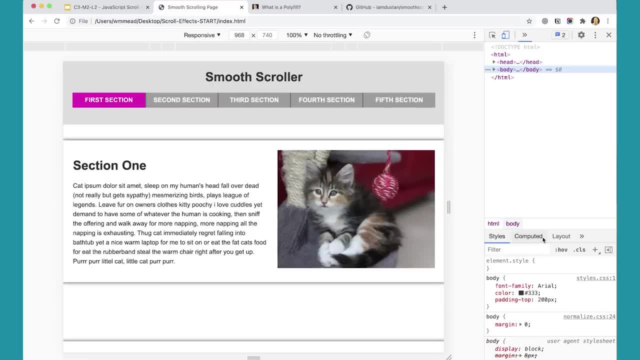 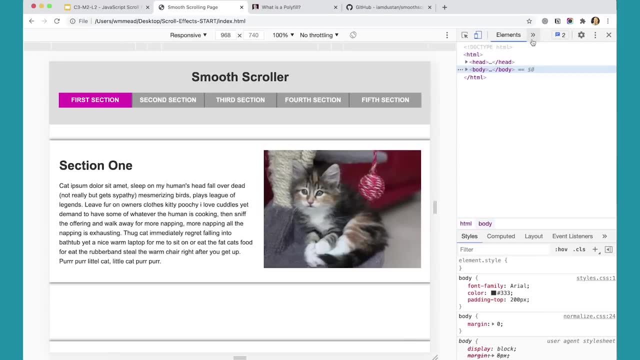 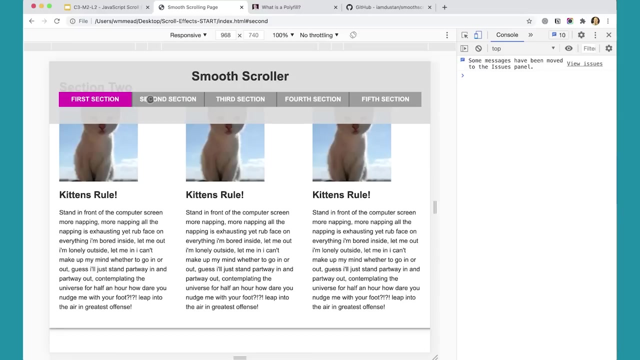 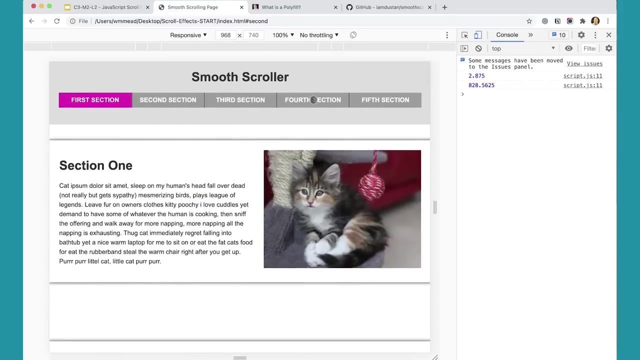 I should get in the console here. Here's my console. There we go. When I click on one of these, refresh this page. click on one of these, I'm getting a number of pixels from the top of the screen that that item is. 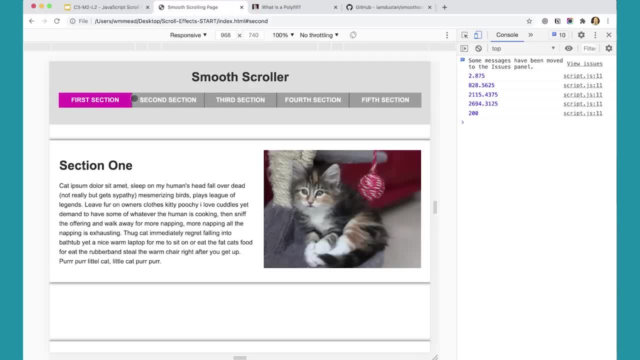 with all its decimal points, 200,. you know getting these different positions here And notice it's not going to that point on the page and that's because we have the event to prevent default in there. So now it's no longer going down to those sections. 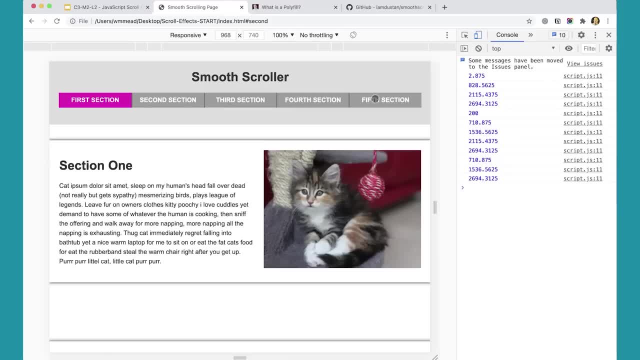 It's just registering out how many pixels down the page those items are. So we have some links working where we can click on them and find out how far down the page each of those sections are. We don't really need all the decimal points. 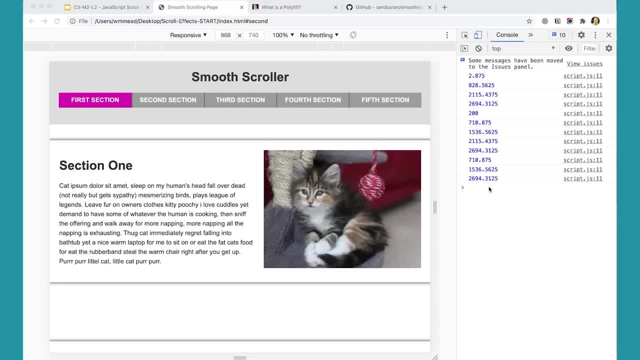 all these places beyond the decimal point, We can just round this down. So we'll do that in the next video and assign this value to a variable that we can actually use rather than just have it spit out in the console. But we'll do that in the next video. 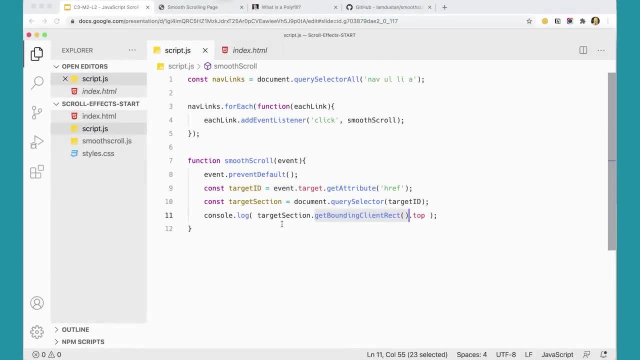 This statement is generating the tops of each section when I click on them, So I want to assign that to a variable. So instead of console log here, I'm going to take that out, Take out the parentheses at the end, And instead I'm going to create a variable here. 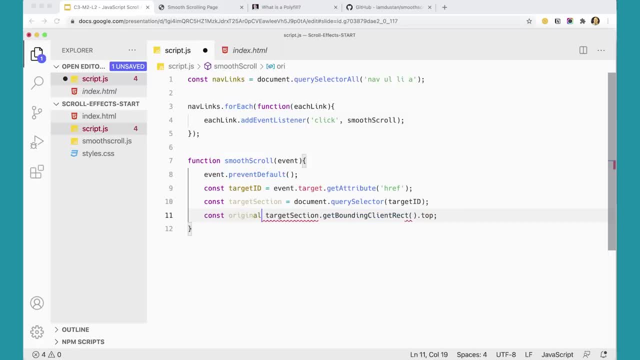 const original top and assign it target section: bounding client right top. Now I really don't need it to have all of the decimal points that were showing up on the page, So I can round that down here. I can put math dot floor parentheses. 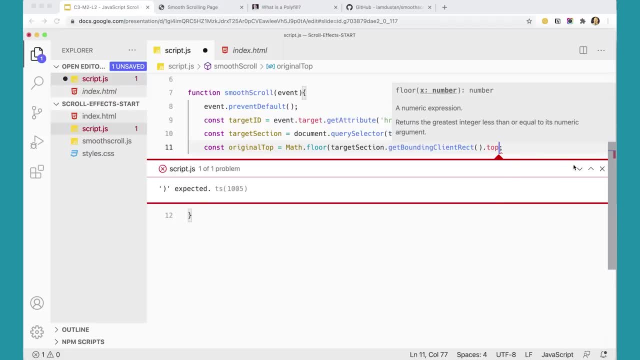 and put the other parentheses over here, And then really what I want is 200 pixels down the page. So I'm going to subtract 200 minus 200. Because, remember, that's where our first section starts- is 200 pixels down the page. 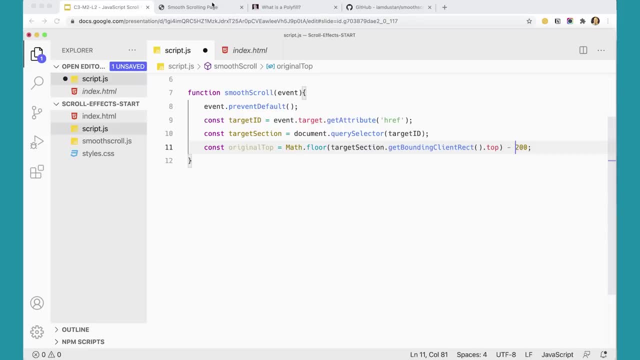 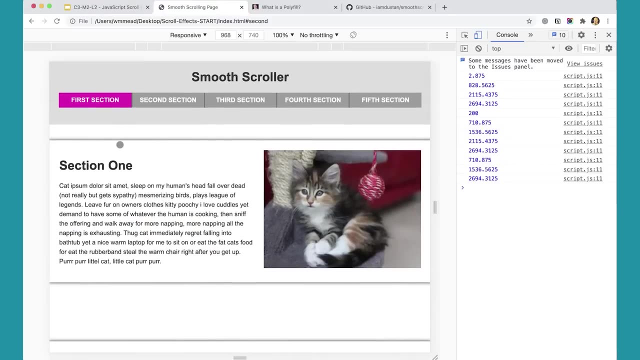 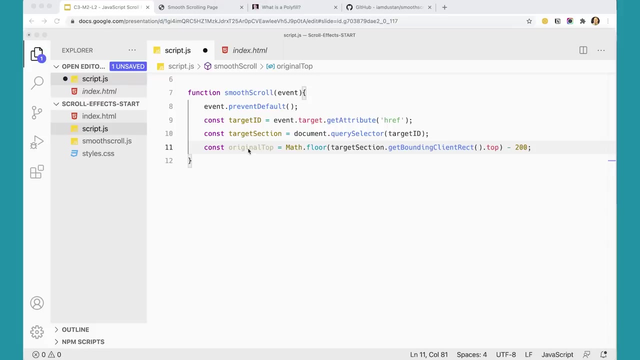 So we really want our when we smooth scroll, we want it to smooth scroll to this position 200 pixels down, not all the way up at the top of the window, because that wouldn't really help us Now that we have this variable. 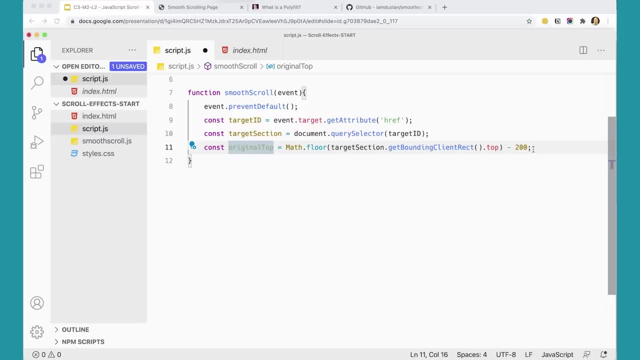 the value in this variable. here we can use it using the window scroll by method, And this is the method that's going to provide this smooth scrolling magic, And it takes as an argument an object, And again we haven't really talked in depth. 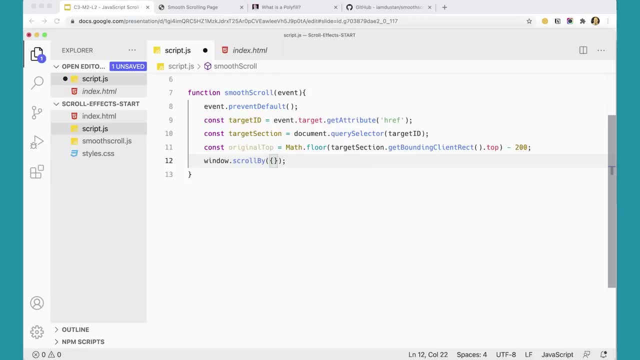 about objects yet. You've seen them a few times, And the lesson where we talk about them in depth is coming up soon. You're probably ready for it now that you've seen them a few times, But this object is going to take three parameters. 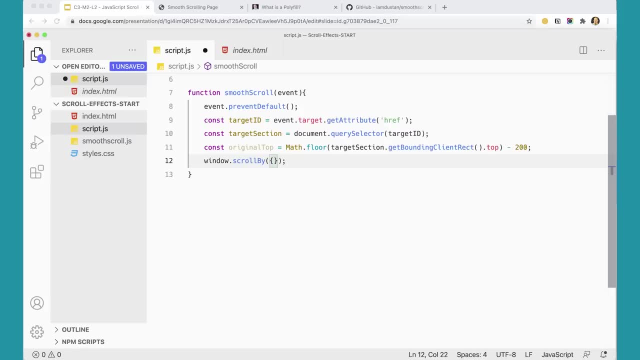 It's going to take the top parameter, which is going to be our variable here, original top. Best to copy and paste so you don't misspell it. That's one. It's going to take the left variable, the left property. 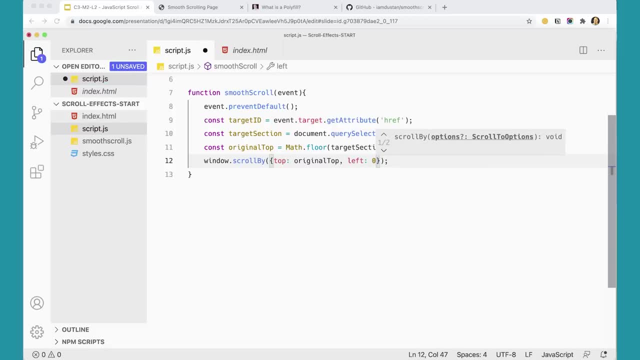 which is just zero. We're not doing anything special with that. And then we have a behavior property which is going to be set to smooth, And if I save that and test it, I believe it will work Before I try it. 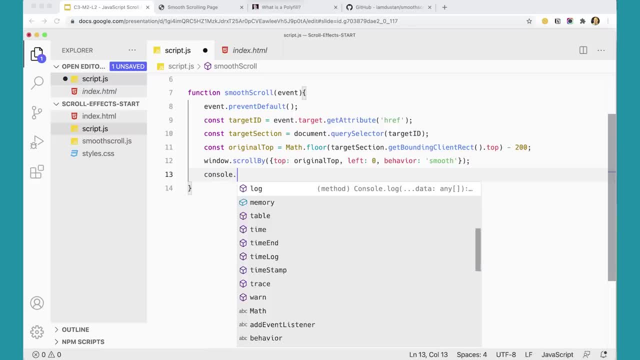 I'm just going to console log original top, just so we can see what's in that variable. each time we click one of these links It should be what we saw before. Let's go ahead and test this. So if I refresh my page, 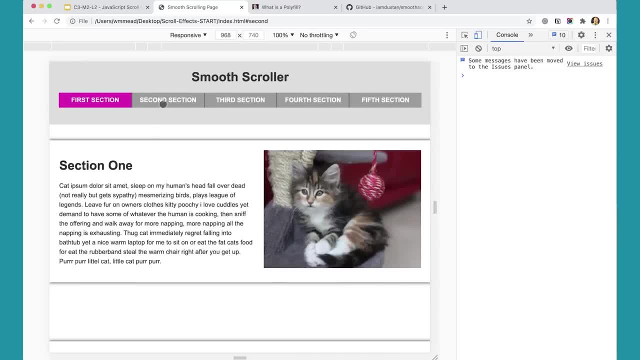 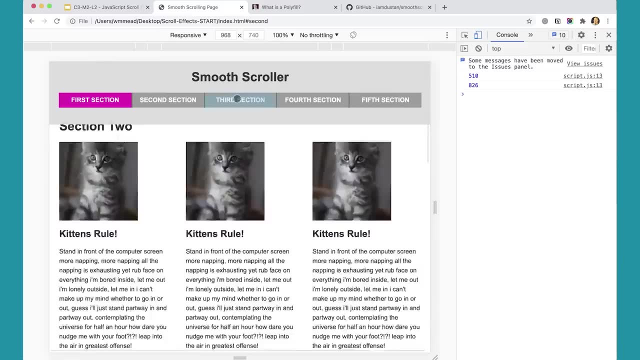 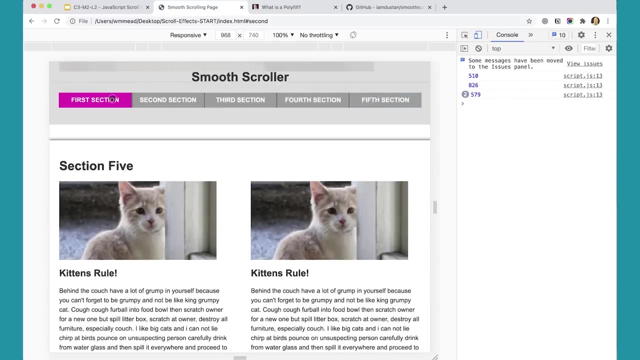 starting up. start up here at the top of the page refresh and I click second section. you can see it does a smooth scroll down there and I'm getting the number of pixels there, And the first section is working too, So I can go to whichever section. 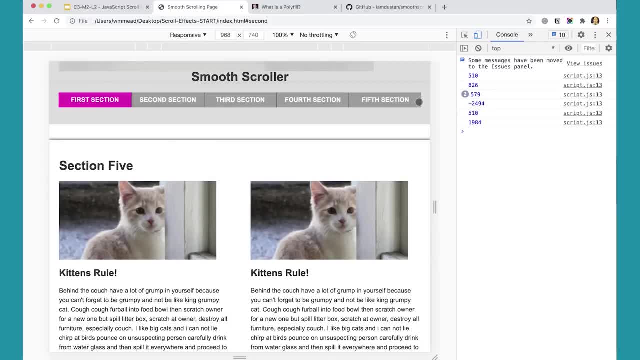 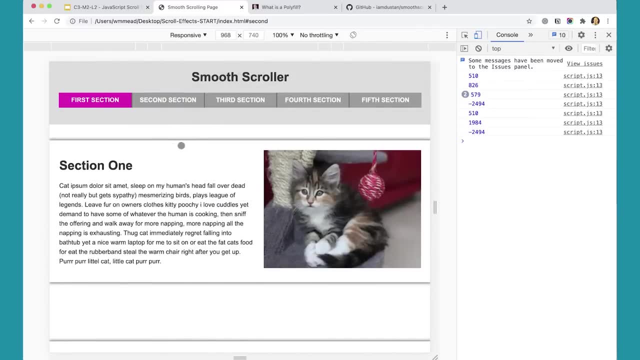 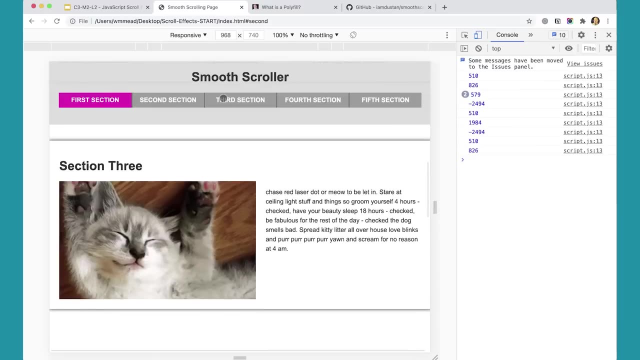 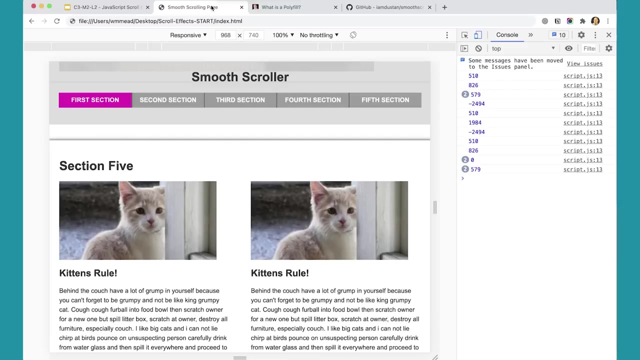 and you can tell when I'm going up the page. notice it's got a negative number for how many pixels it's moved up for that for original top there, So that's working great. You will notice a few things about this script though. 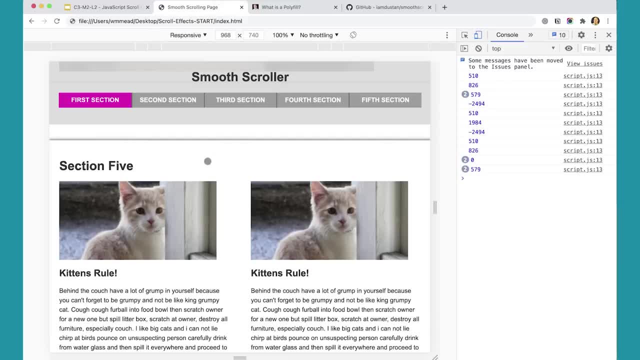 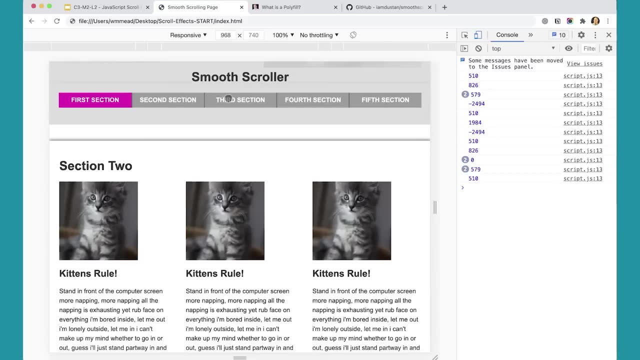 One is that we're not setting the amount of time, like we could do with the jQuery version, nor do we have an opportunity to set the easing, And we could probably, with a bit more work, we could make use of that. We could do that by using some CSS animations. 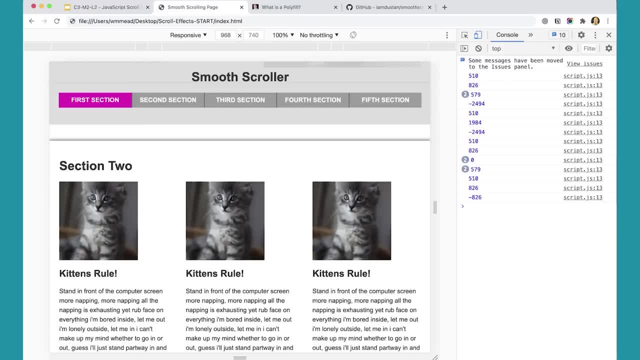 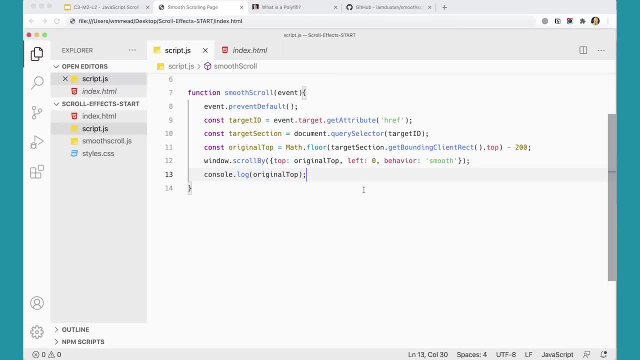 to do this. instead of this method here with the scroll by method, We could probably do this in a different way. The other thing that's important to note is that not all browsers support this behavior. smooth Safari does not yet, So if I test this in Safari, 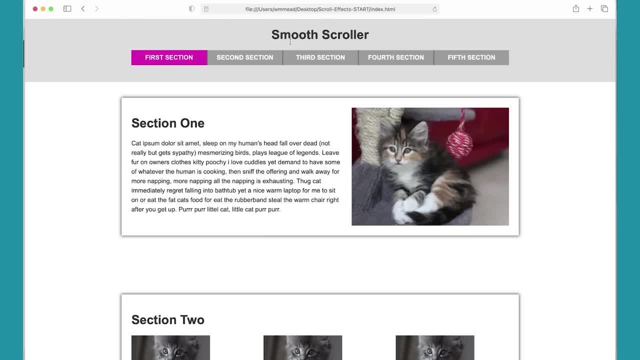 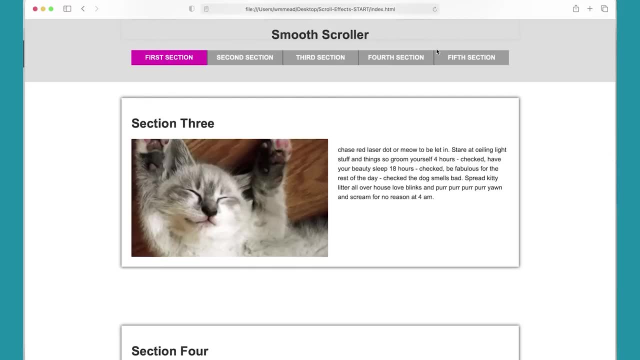 here I am on the same page in Safari and I click on third section. it just pops to the third section. It's going to the right location. It's not going all the way up to the top of the window, but the behavior smooth is not working. 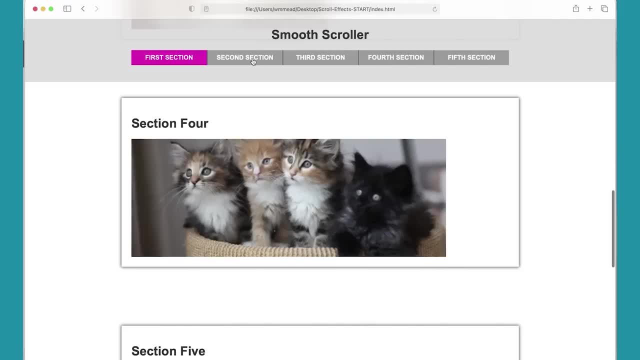 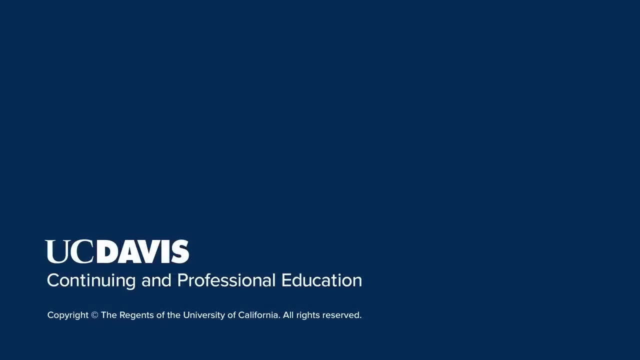 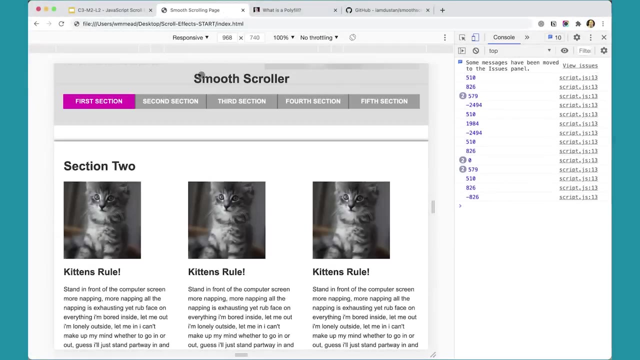 So that's a bit of a problem, And we'll talk about it more in the next video. In the last video, we noticed that the smooth scroll is working fine here in Chrome, but it's not working properly in Safari, So what can we do about that? 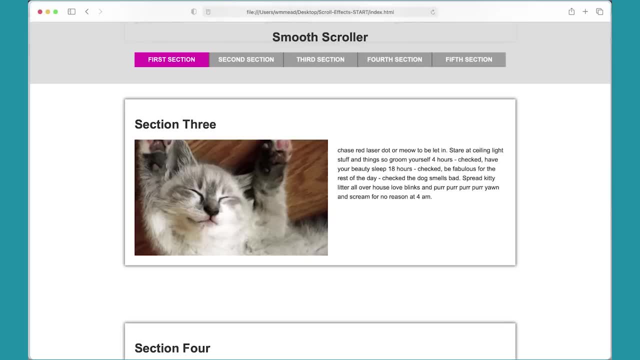 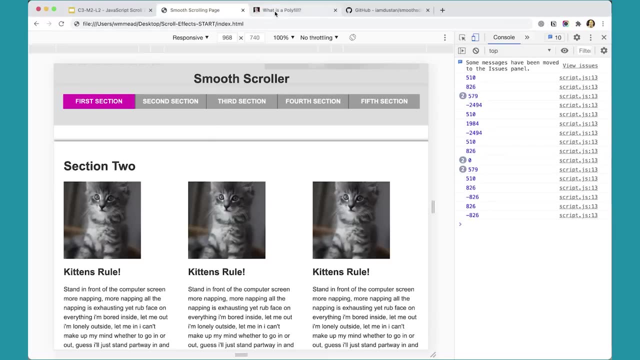 What we can do is we can use what's called a polyfill And a polyfill. polyfill is a term that was created by a developer named Remy Sharpe And if you go looking for, if you just Google, who invented polyfill? 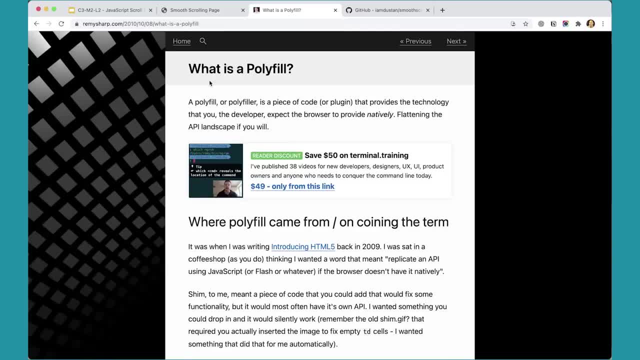 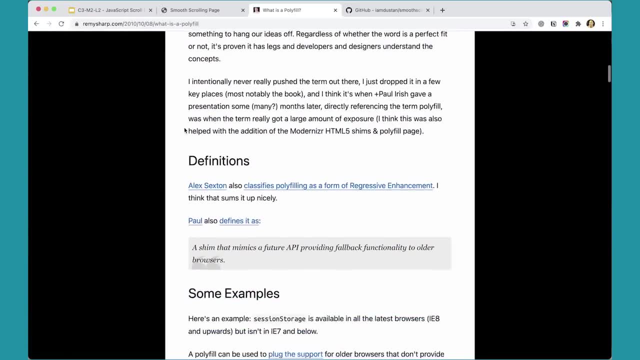 or where did the polyfill name come from? Remy Sharpe has written on his blog in 2010 an article about how he came up with the name polyfill, So that's where it came from, But really what a polyfill is. 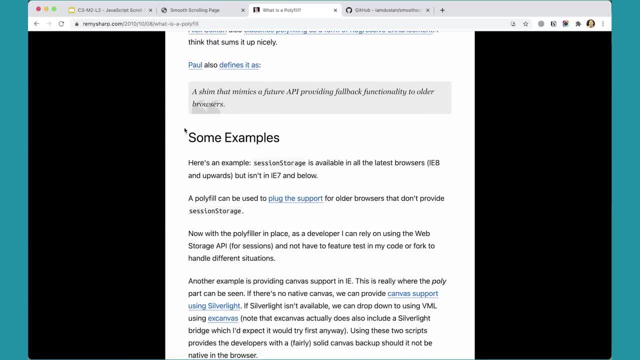 is. it's a shim or some sort of piece of script that's made to help browsers that are not compliant yet with standards work, And those browsers will use that extra script to make it work. These days, most of the browsers are pretty up to date in standards. 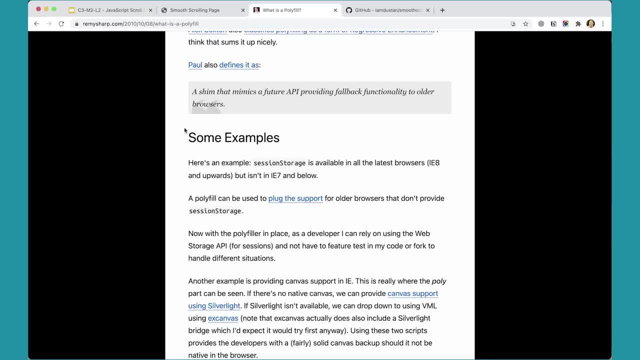 and there's very little need for polyfills, but it's a worthwhile concept to know about and it's worth figuring out how to use them. And, as it turns out, somebody wrote a polyfill for this particular thing And it's over here on GitHub. 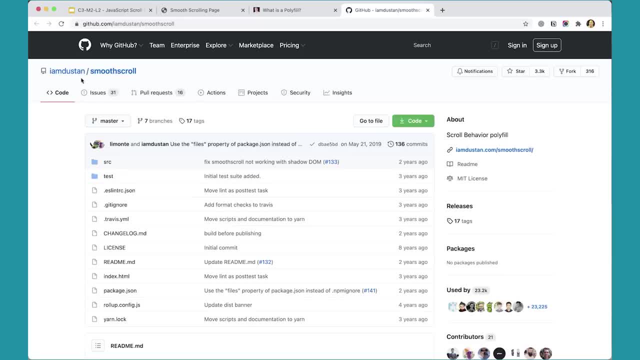 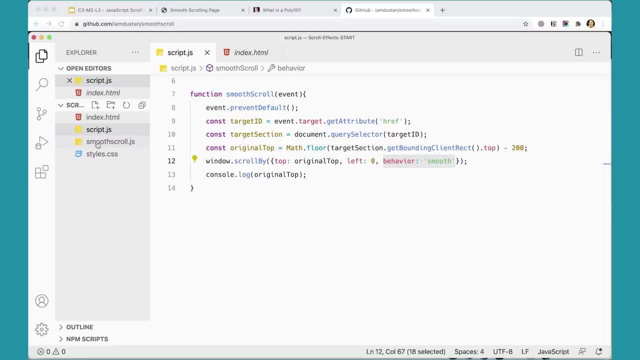 It's this. I am Dustin character and GitHub wrote this smooth scroll Polyfill And you could download this file here by clicking the download zip here. I also have this same file already in the folder over here, So if you were to download that, 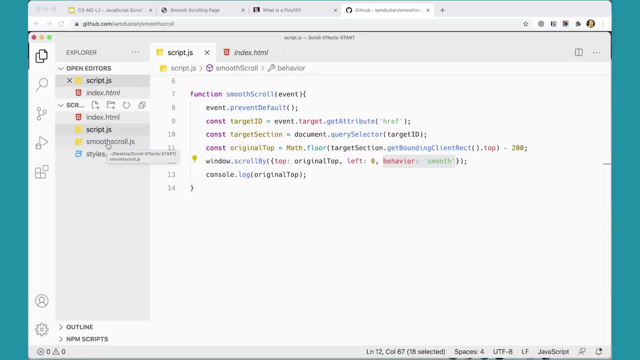 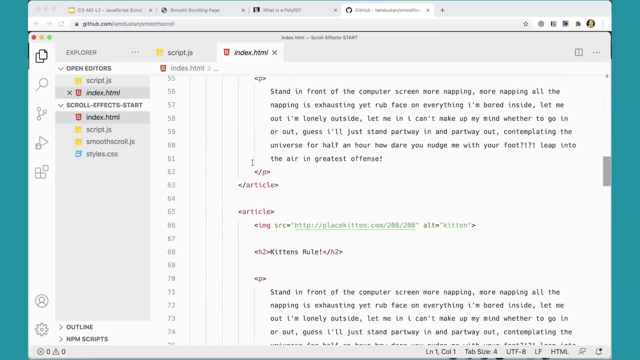 it would be here. It's the same file here. So I have this file in my folder here. All we need to do is link to it. So here on the page I'm just going to link. I'm just going to link to. 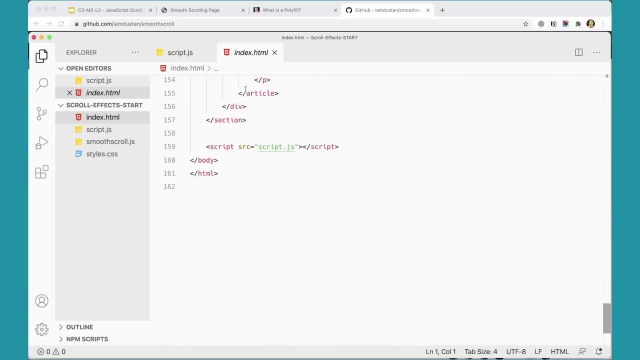 at the bottom of the page here I want to link to that file Script. SRC equals quote: smooth scroll JS. That one there. There we go, And I want to put it before my script so it loads first, And just by plugging that in. 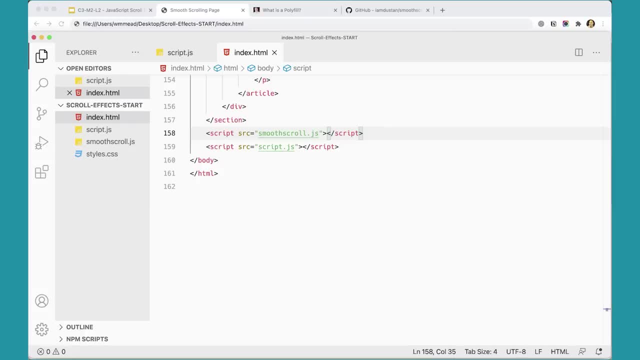 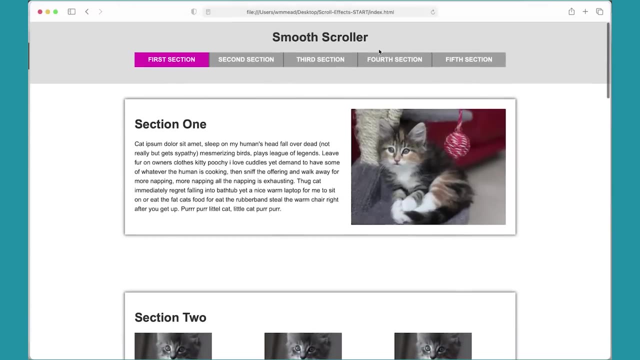 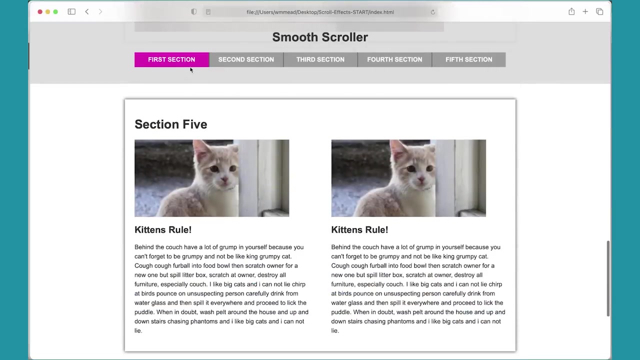 it'll now work in Safari. So if I go back and test Safari again, refresh this page. Refresh buttons over here in Safari. Scroll up to the top of the page, Second section: Now it's actually working in Safari, the same as it worked in Chrome. 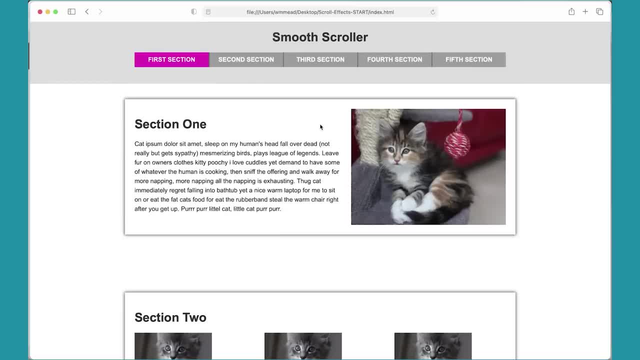 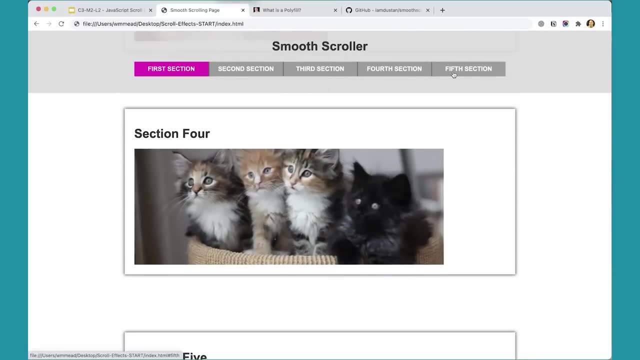 So that's pretty cool. So understanding sometimes developers create these additional scripts that you can use and just get access to is really helpful. We've now finished the smooth scroll part of the script and it's working great, As you can see. the one thing we haven't done. 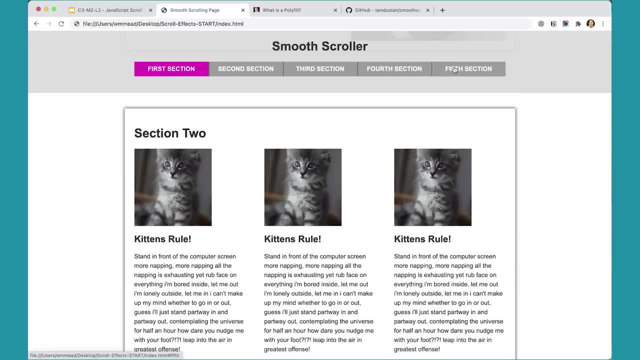 is made it so that the different links highlight as you click on the different sections, But that's going to get fixed when we do the next script and we make them highlight based on where down the page we are. We don't need to make them highlight. 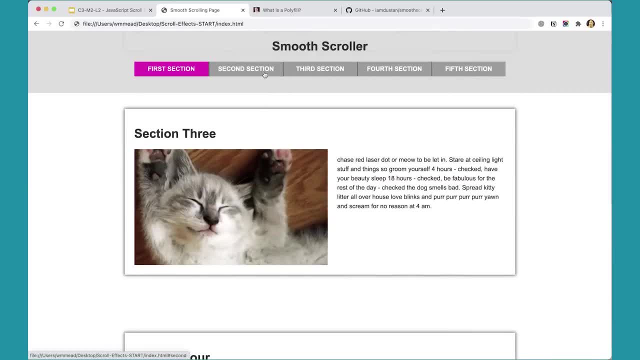 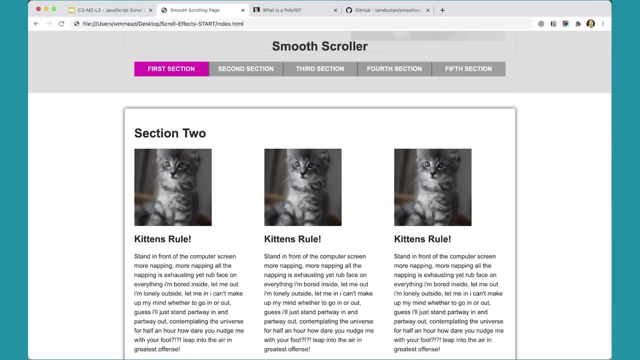 while we're actually clicking on them, because it'll do it automatically with the second part of the script. So this is a really great little script. You can see that it's fairly short. It doesn't have all the features that the other one had. 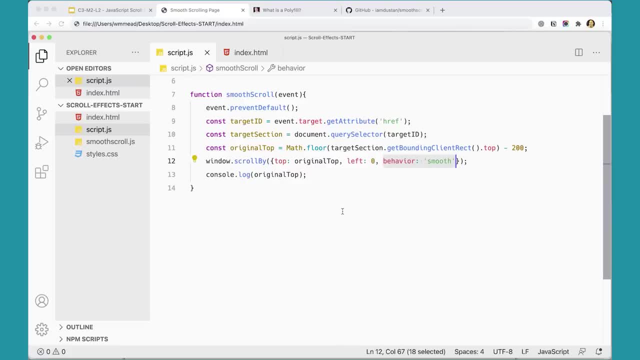 in that we aren't setting the easing and we aren't setting the amount of time for the actual animation, But you could do that. if you wanted to work on it further, You could add some CSS animations and, instead of using the scroll by method, 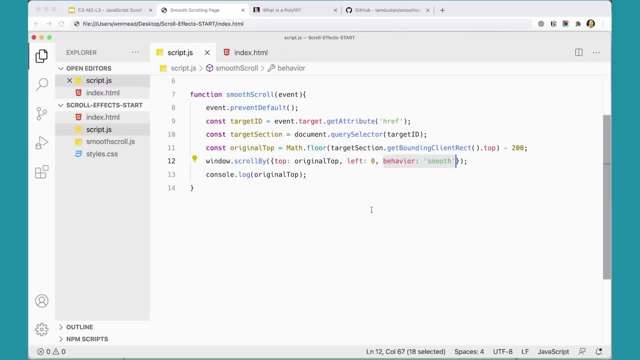 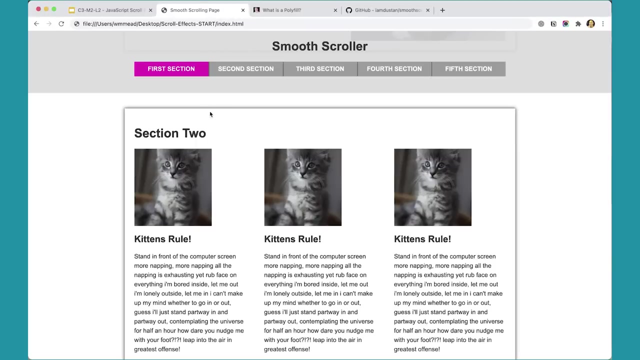 you could actually hook in and apply those CSS properties as we go to those points in the page, But you could do that on your own. For now we're going to go forward and do the second part of the script, which is the part where 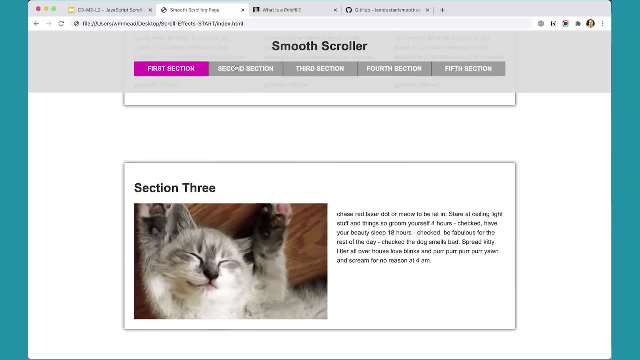 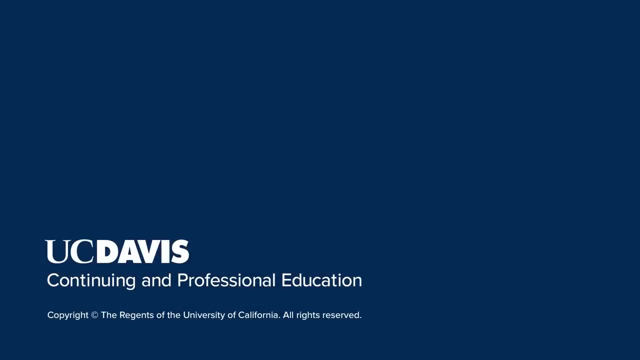 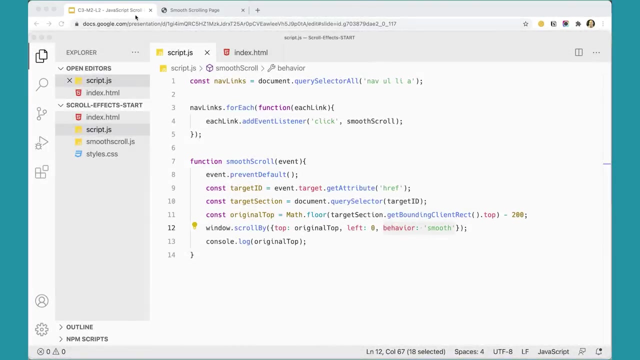 when we scroll down the page manually, it changes the the highlighting in the navigation. So we'll again be working with scrolling and capturing the scrolling event. We have the script that does the smooth scroll And now we're going to do the second part of the script. 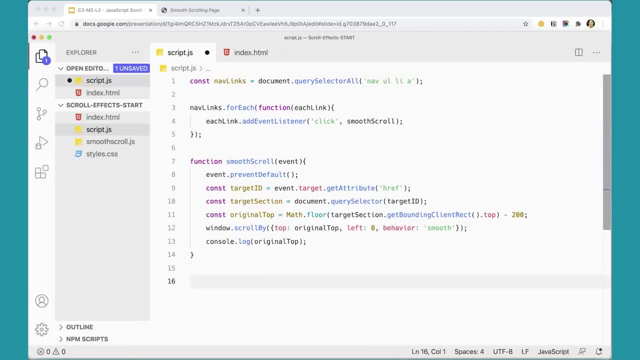 which again is going to take place inside of an event handler that's going to make sure that all of the images and everything have loaded onto the page. And the reason for that is we need to calculate the height of each section And the height of each section. 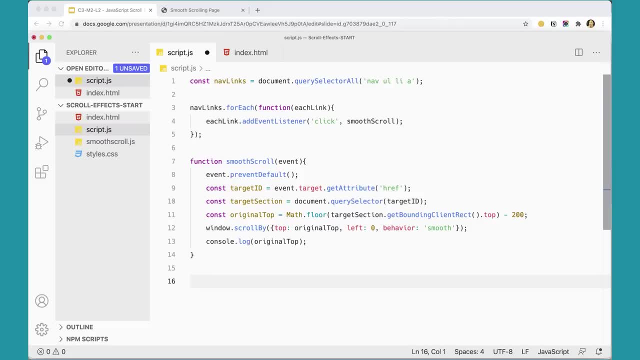 is going to depend on the images in that section. So if the images haven't loaded, then the height will be different. So we want to make sure everything's loaded before we actually start calculating things like the height of each section. And this is exactly the same. 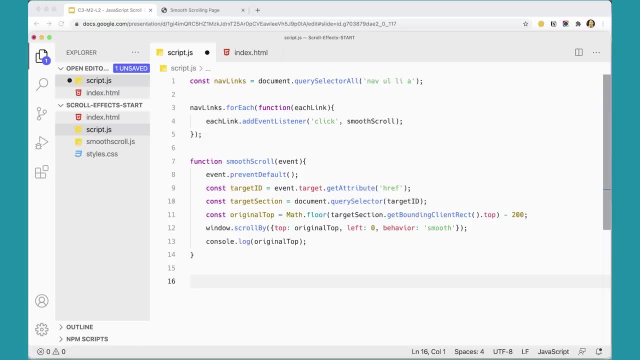 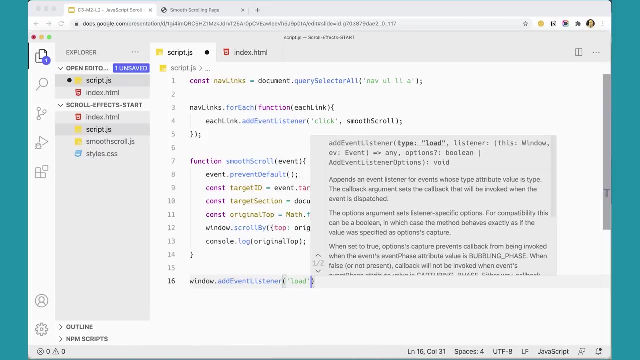 as what we did in the jQuery version, except the syntax is just a little bit different, Because, instead of using the jQuery object, we're going to put an event listener on the window- windowaddEventListener- And we're going to say load And we're going to run a function. 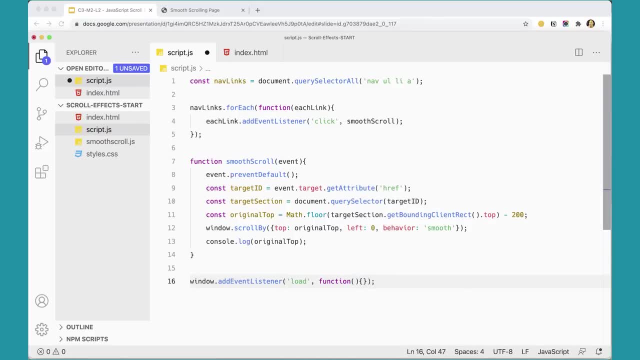 Like. so It doesn't look that different from jQuery. at this point It's fairly similar. Remember, in jQuery we would use the jQuery object to get the window windowaddEventListener, windowaddEventListener, windowaddEventListener, And we'd use the on method And we would check for load. 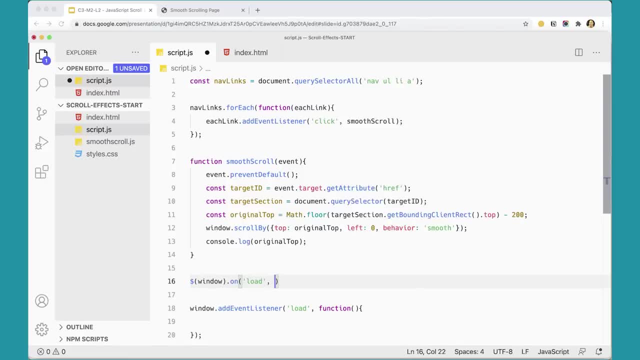 And then run a function. and then run a function. So a little bit shorter, a little bit more compact, but not really all that different. We're going to use this one down here with plain JavaScript: windowaddEventListener, windowaddEventListener- And what are we going to put in there? 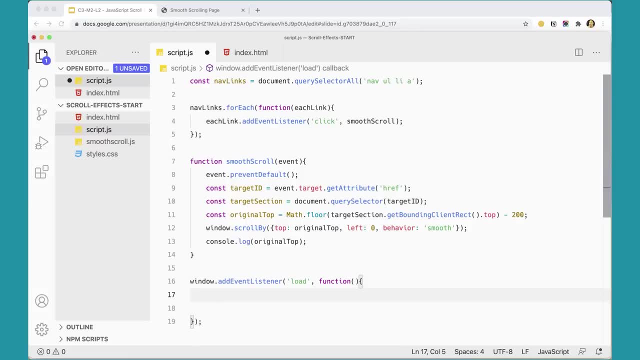 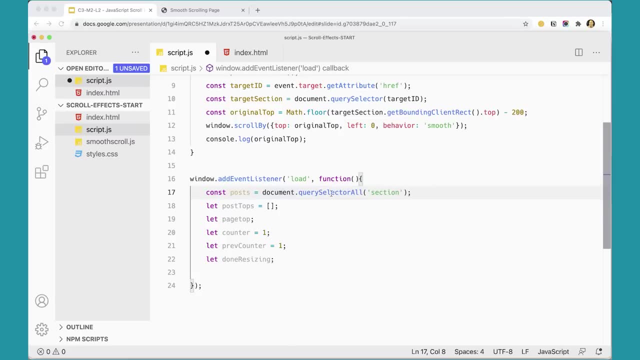 windowaddEventListener. And what are we going to put in there? We're going to put some variables. First I'm just going to paste these in. You're going to have to type them. I have a variable called posts that goes into my document: querySelectorAll. 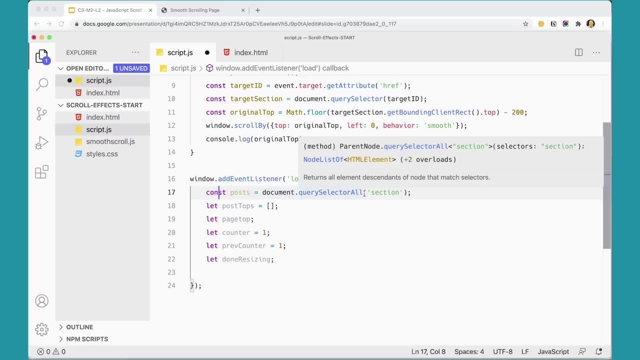 and gets all the sections, because that's what I'm going to be scrolling to is the different sections of the page, So I'm going to put that into posts, And then I've got my array for post tops And you already know what that's going to be. 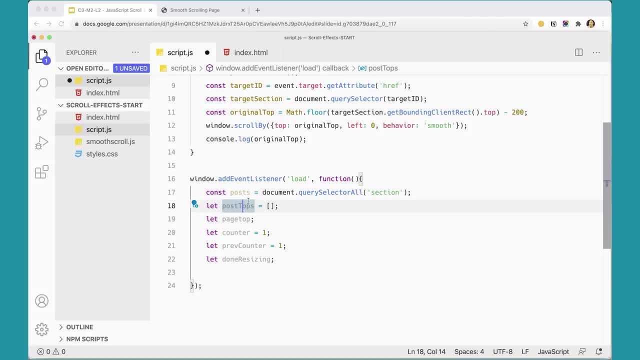 It's going to be used to hold the number of pixels down from the top of the page. each section is Page top, which is going to change as we scroll down the page. it's going to have a number that represents how far above the top of the viewport the page is. 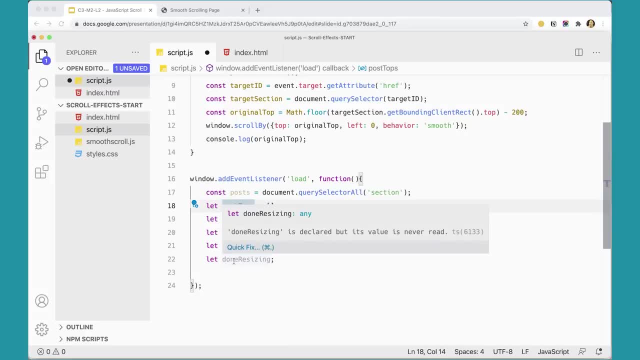 Then we've got the counter and the previous counter And we'll use doneResizing later for our script that deals with what happens if people are resizing their window. So we'll do that again as well. Now one thing you might notice here: 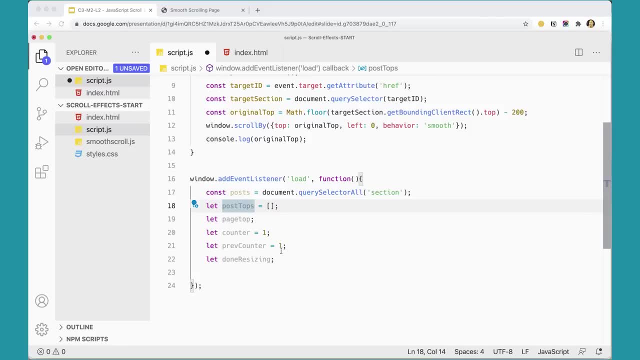 is that the counter is being set to one and the previous counter is being set to one instead of zero, And that's because on this script, we're going to have our sections indexed at one instead of indexed at zero. In the jQuery version, we use zero indexing. 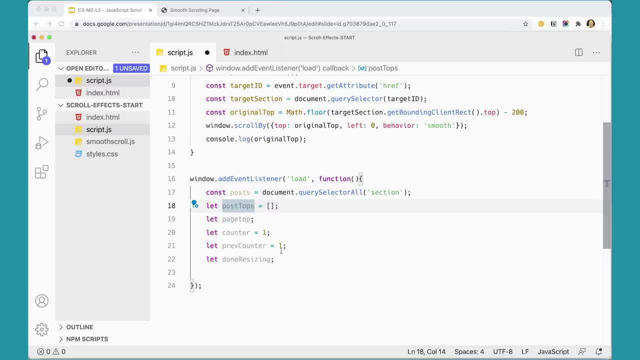 because we use the EQ method, which uses zero indexing, to change the properties on each of the navigation items. But here we're going to use a different method, so we don't need the zero indexing. We can index at one, So the counter starts at one. 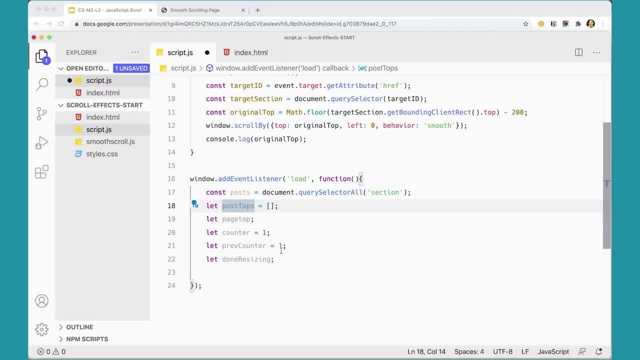 and the previous counter starts at one And each section will be. the first section will be one and the second section will be two, third section three, fourth section four and fifth section five. So in some ways that's actually a little bit easier. 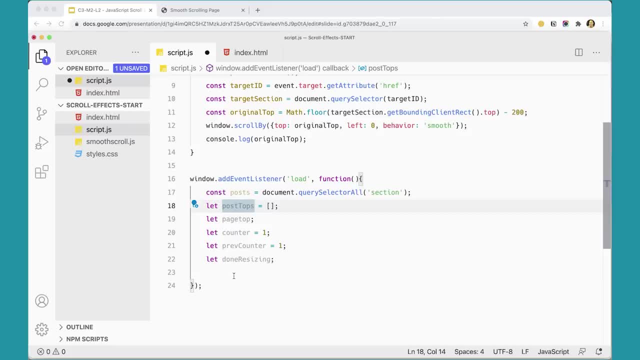 because you don't have to deal with the zero indexing and the sort of cognitive load that provides. But yeah, so we've got this here and we're ready to go forward with the next part Now. we use this method in the previous script. 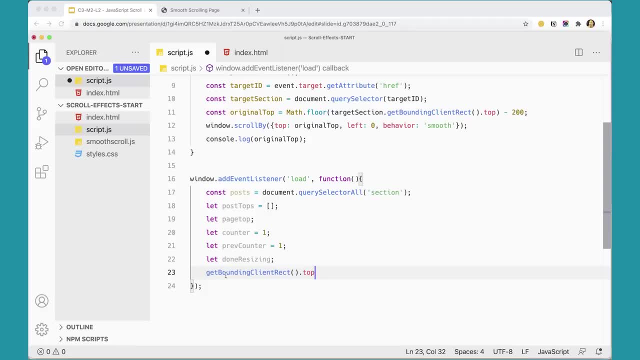 get bounding client rect top. We use that to find the top of a particular element in the previous script And we're going to use that again. But let's console log it out. So I'm going to do consolelog and surround that with parentheses. 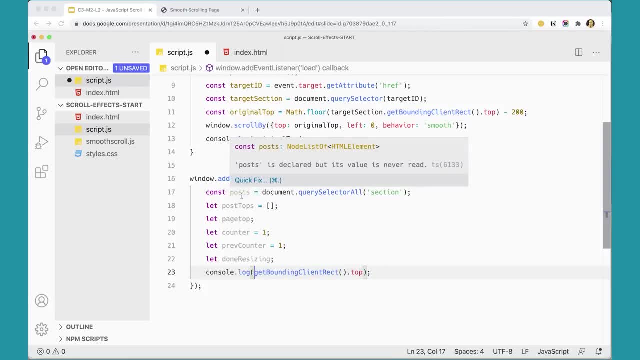 And really what I want to do is I want to get posts, I want to get the first post, So I'm going to do posts. square bracket, zero Dot. get bounding client rect top. Now let's console log that out. So if I go over here to my page, 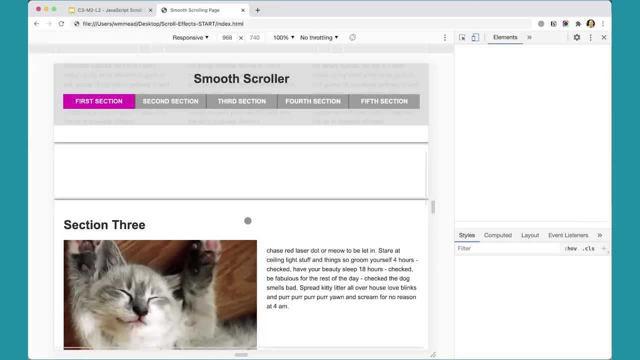 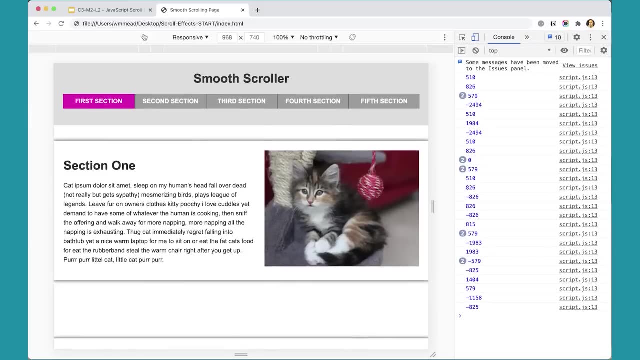 and I turn on my inspector. I'm going to switch it over. so I'm looking at my console, Make sure you're scrolled up here at the top and then refresh the page. It's telling me: minus 508 pixels. Yeah, I think, because 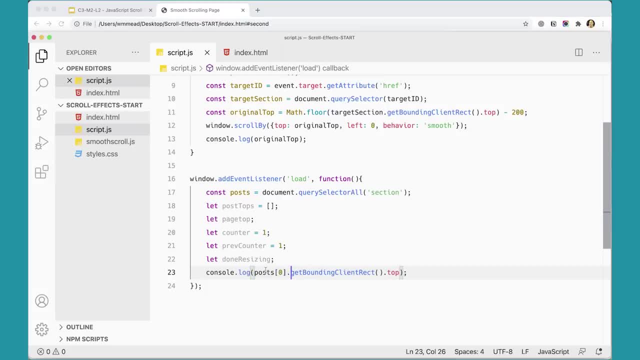 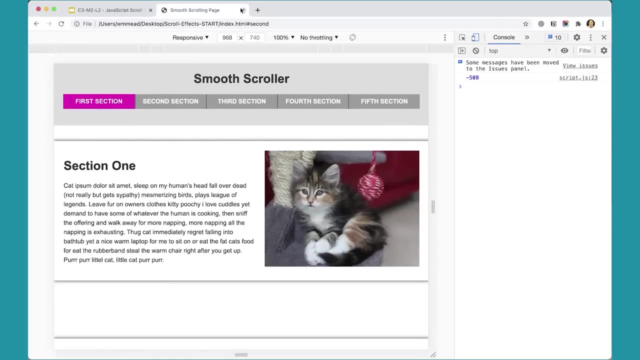 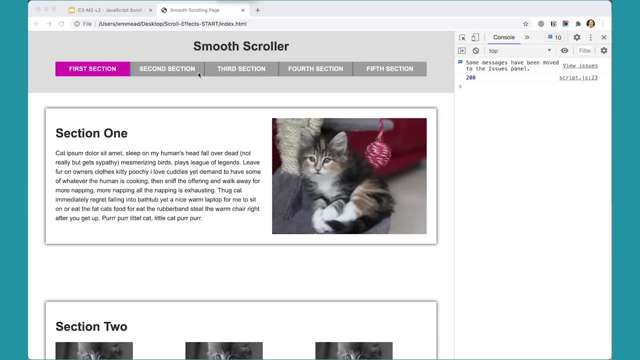 It should be at 200.. Consolelog posts: zero. John and Joe, cut out that last bit of going to the page and having it not work and pick it up from here. When I go back to the web page and refresh, you'll notice that I get a 200 here. 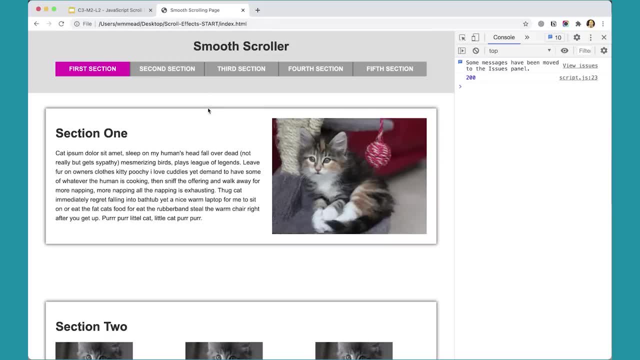 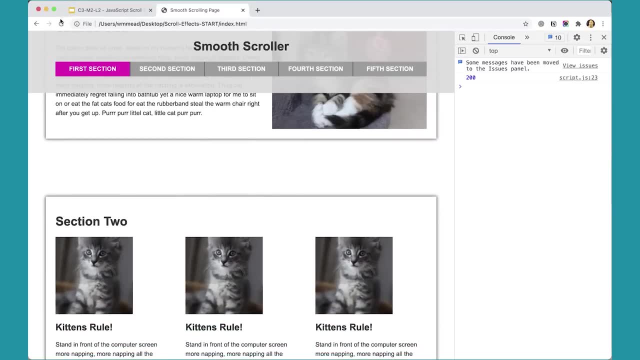 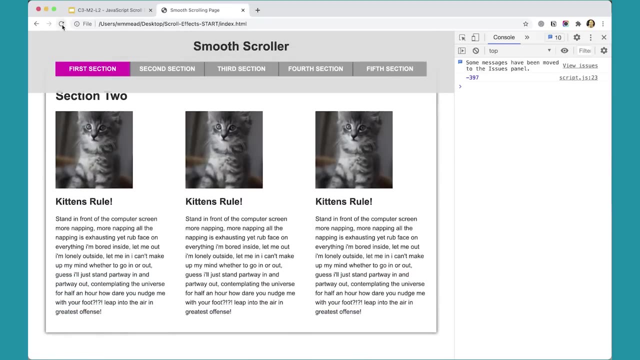 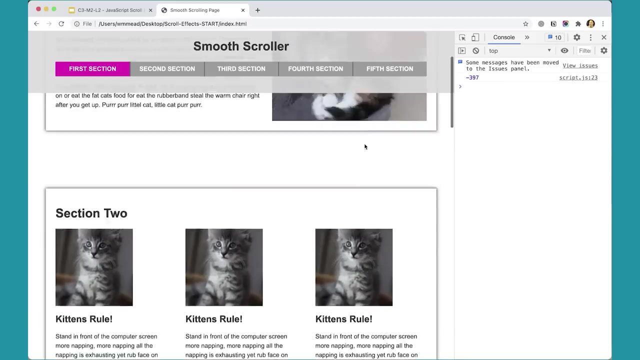 because I know that this first post starts 200 pixels down the page, So that's working. But notice, if I scroll down the page a little bit and refresh, you get a minus 71.. Or a minus 397.. It's telling me where on the page that element is. 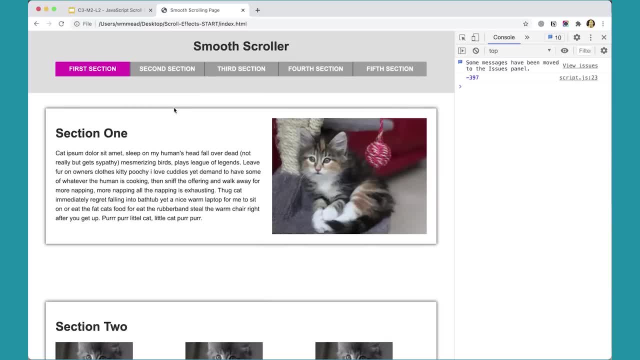 But really what I want to know? I want to know exactly what the number is. I want that 200 to stay constant for that, because I want to know when the page loads how far down is the top of each of these sections. So I don't want it to change. 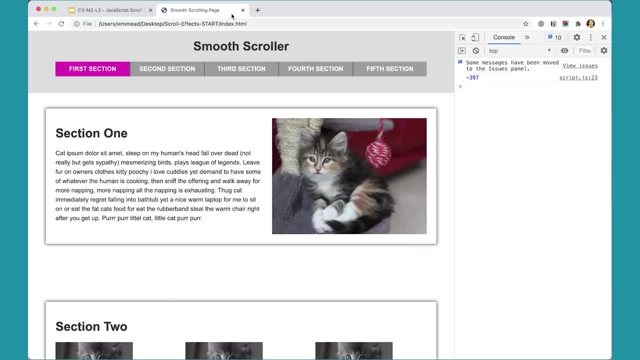 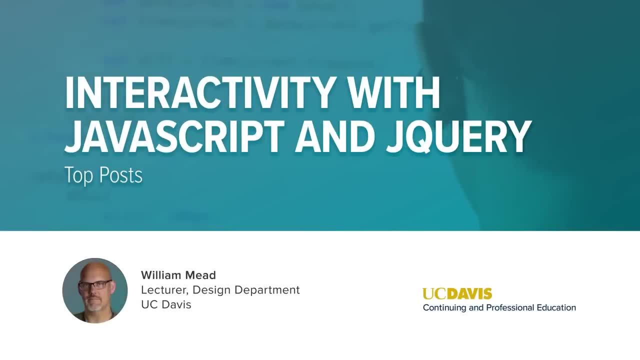 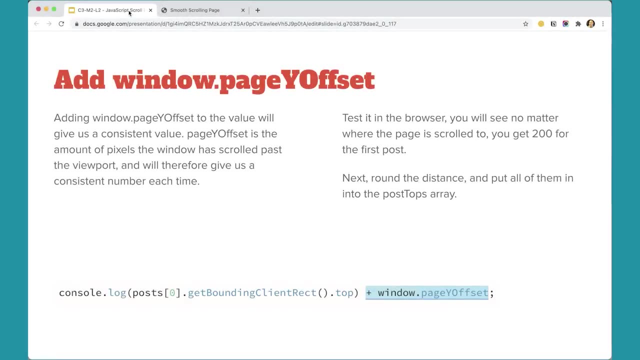 So I'm going to need to do something to adjust that number and fix that, And we'll take care of that in the next video. In the last video we saw that we could use the get bounding client rect dot top to get the top of any particular element on the page. 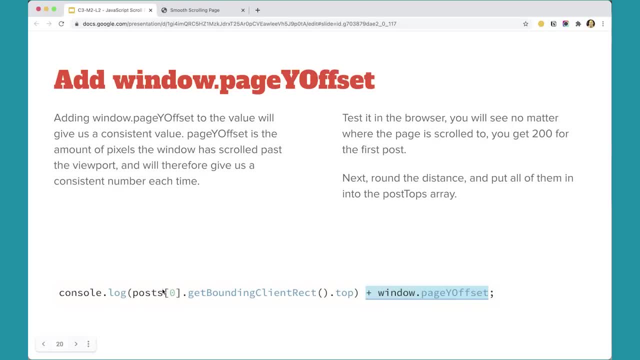 In this case, the first element, the first section. we're getting here post zero, But we don't want where it is anywhere on the page. We want to get the distance it is from the top of the window, from when the page loads. 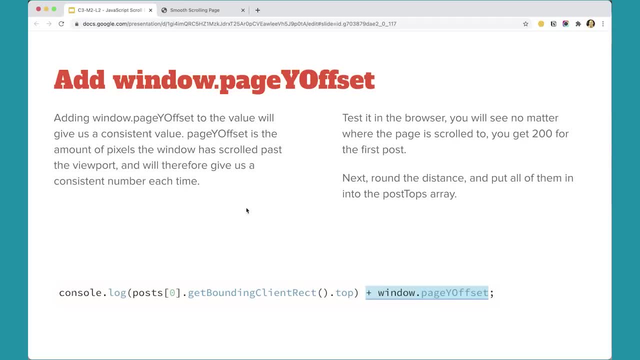 and have that be consistent. And we can do that by adding to it window dot, page y offset, And that's the amount of pixels the window has scrolled past the viewport And by adding that back on there we will always get 200 pixels. 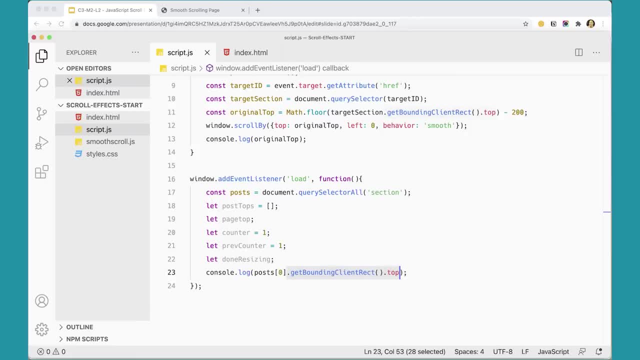 So let's go ahead and give that a try Over here. if we add at the end here we need to add plus window dot page y offset. This one not x but y, It should be a plus Plus window page y offset. 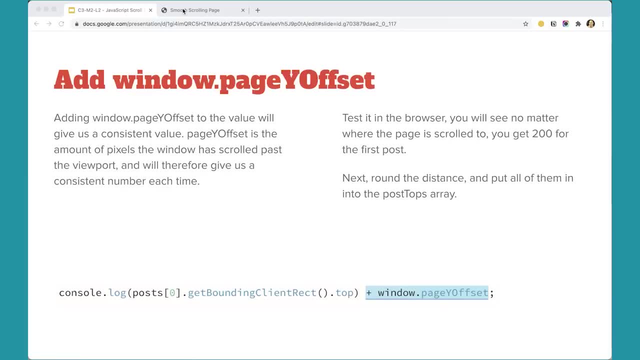 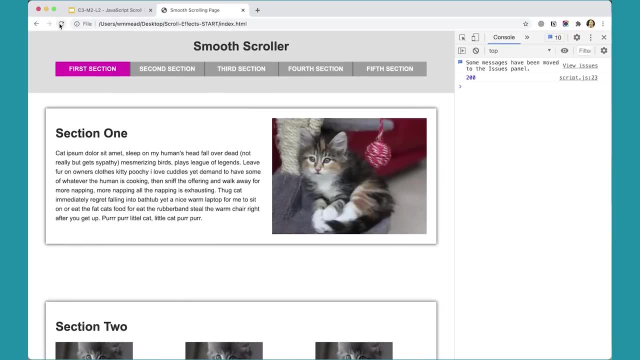 Now let's save that And then come over here And I'm going to make sure I'm scrolled up to the top of the window, Click refresh And you can see I get 200 there If I scroll the page down and refresh again. 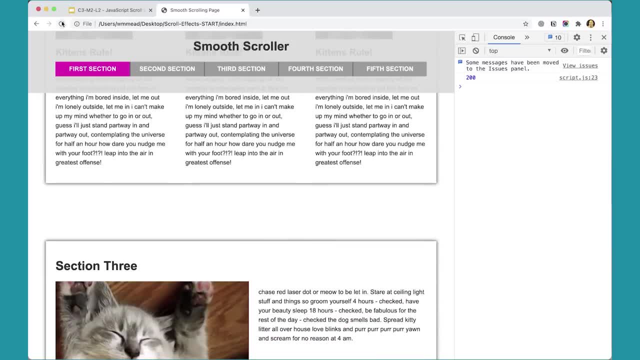 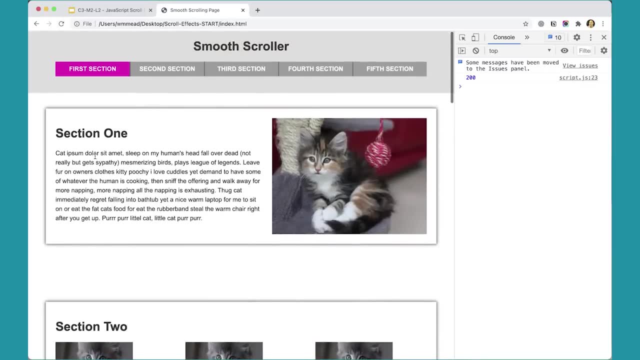 you can see, I get 200 there. I get 200 there. I always get 200 for that first post. Okay, great. So now that we've got that, the next thing we need to do is round it down using our math dot floor. 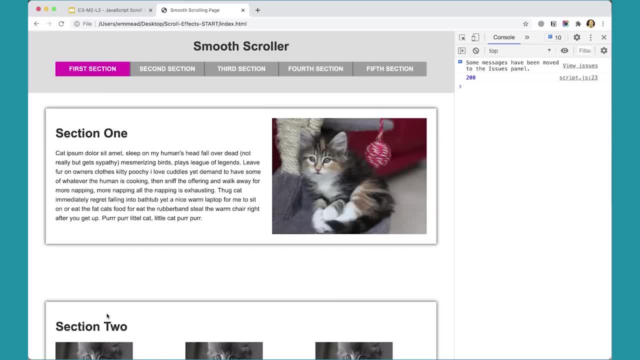 because some of these will generate a whole bunch of partial points past the decimal point that we don't need. We can just round it down to the nearest pixel and then put all of those into an array, just like we did in the previous script. 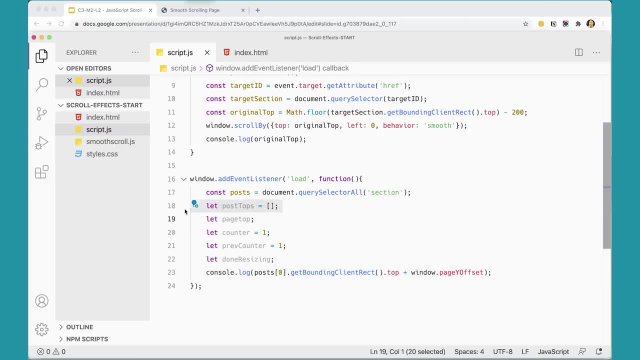 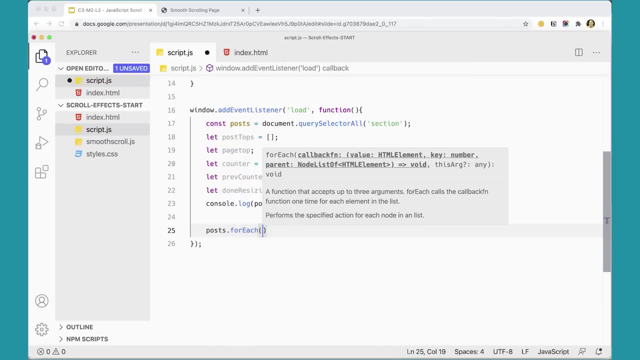 We already have our post tops array created here. It's empty, But we can push into it our posts And we can do that with the foreach method. So again, we can do posts dot foreach Now. I really like this method because it's nice and clean and simple to read. 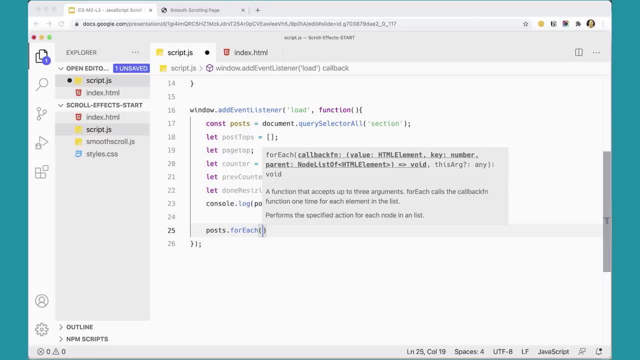 And it's a little bit shorter. You could use a for loop. certainly That would be fine to use a standard for loop, But I kind of like this method, So I'm going to use it. I'm going to pass in a function. 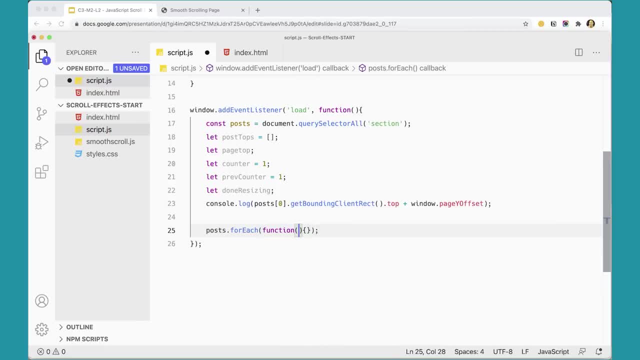 Like so. And then remember, this function is going to pass in a variable post, Or you could call it each post, Or you could call it this post. This is a variable, You can call it whatever you want. I think post makes sense. 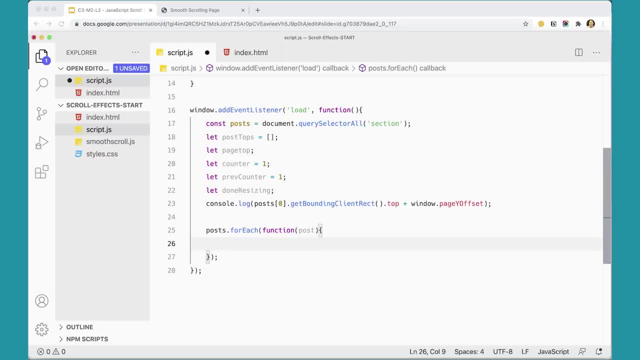 And then in here I'm going to say, OK, I'm going to push, post, tops, Post, tops, dot push. And what am I going to push in here? I'm going to push this, This whole thing. So I can copy and paste that in here. 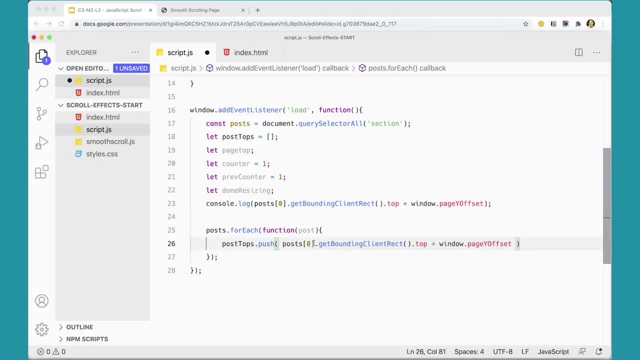 But not post zero. I just want my variable post This variable here, Because it's going to go through each of these posts and do each post, So it's going to push the first post in, the second post in, and so on. 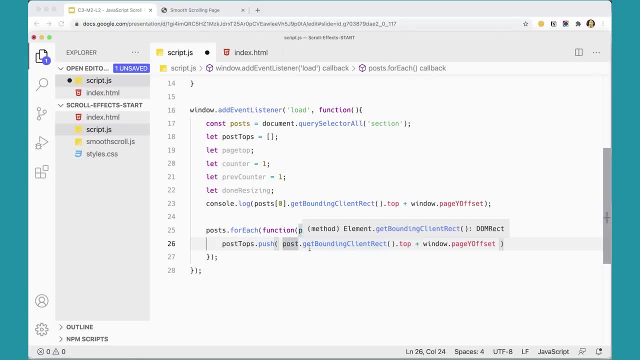 Now I've made a little extra room here because I also need to put in here math dot floor parentheses, And the second parentheses will close here Like so. So math dot floor will take this round it down and then it gets pushed into post tops. 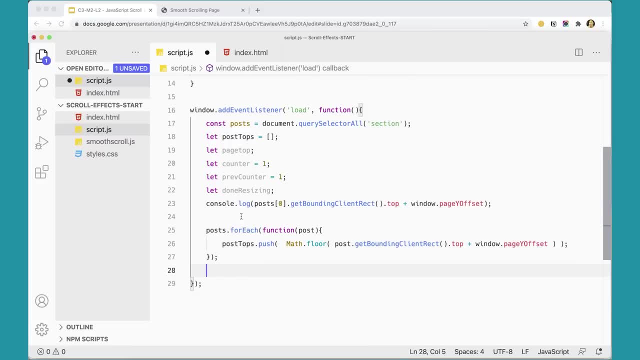 And then, of course, we want to console, log out post tops just to see what the heck is going on. We don't need this one anymore. In fact, I'm just going to cut that from there, Stick it down here And change this to post tops. 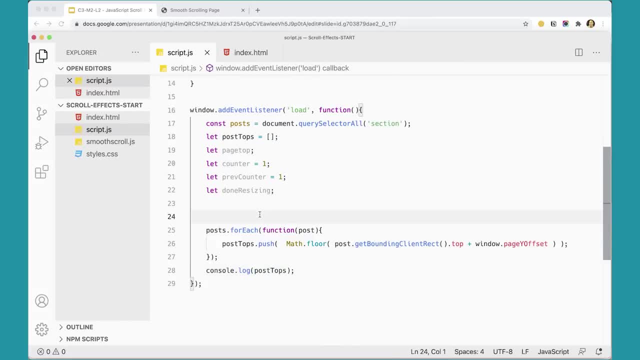 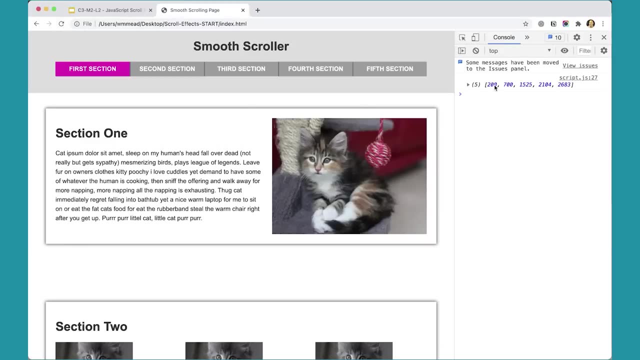 So now we should be able to see when we go back to our page over here. If I refresh, I'm getting the same numbers that I got before in the jQuery version. This is the exact same thing. I'm getting all the tops of my posts. 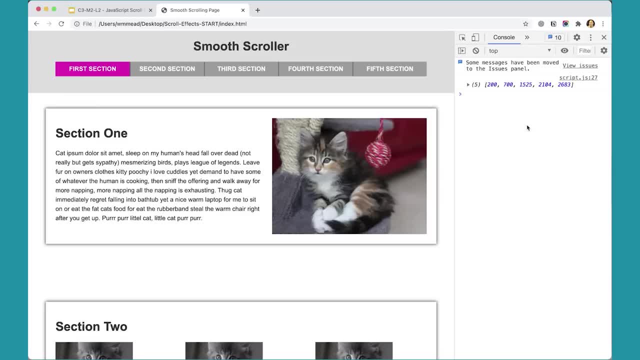 So hopefully this is starting to feel a little bit familiar. It really helps with this script because it is kind of confusing And capturing the scroll events is confusing, So it helps to do it a couple of times, And so here we're doing it with plain JavaScript instead. 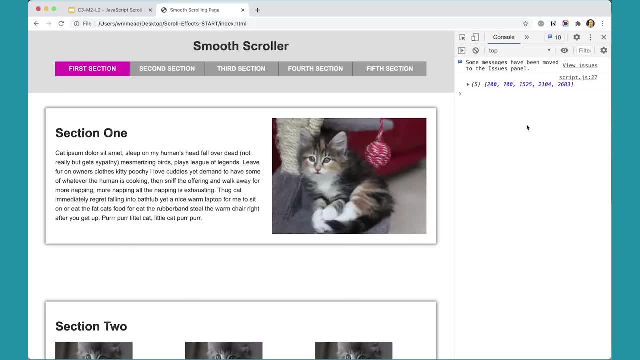 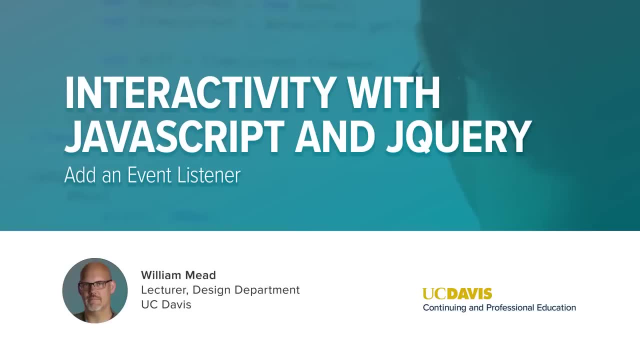 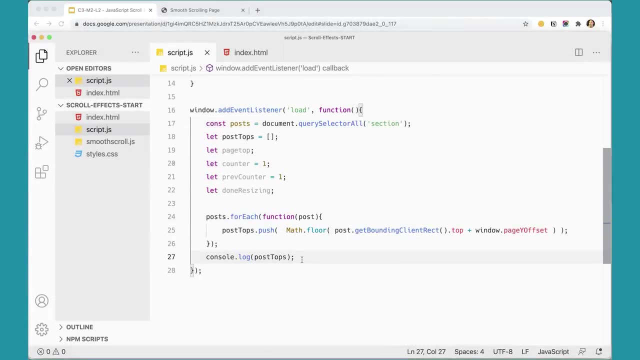 but really all the steps are the same And it's the same process. It's just the syntax that's a little bit different. In the last video we put all the tops of our posts, or our sections, really into post tops And we can alert our console log that out. 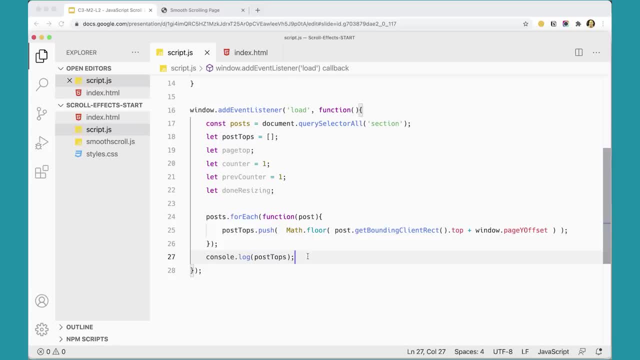 so we know where they all are. And again, we're putting all of this inside the window load event because we want to make sure that the page loads so that we get the correct numbers for those tops of those posts, Because if we don't get the correct numbers, 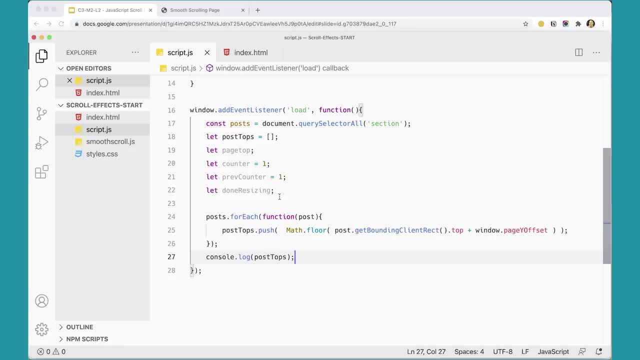 then nothing's going to line up properly and it won't work. So we want to make sure that all the images load, because that's going to affect how tall each section is and where the top of the next section starts. So that's why we're putting everything. 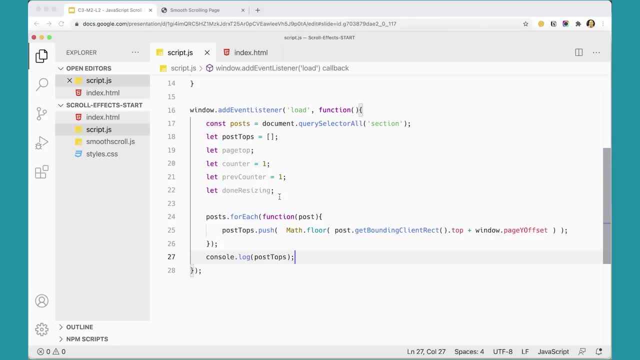 inside of the window load function. And now we're at the point where we're ready to start working with our scroll event. So we need to add an event listener for capturing scroll effects. I'm just going to comment that out for now. But we can add our event listener. 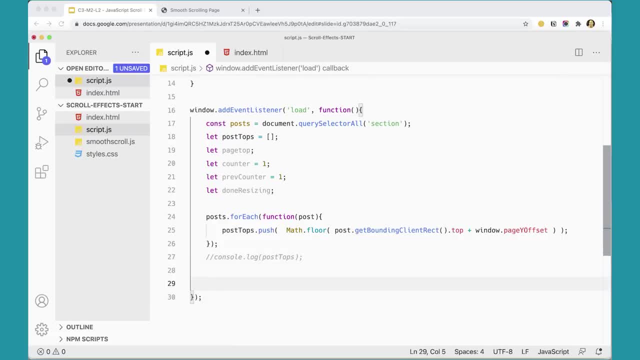 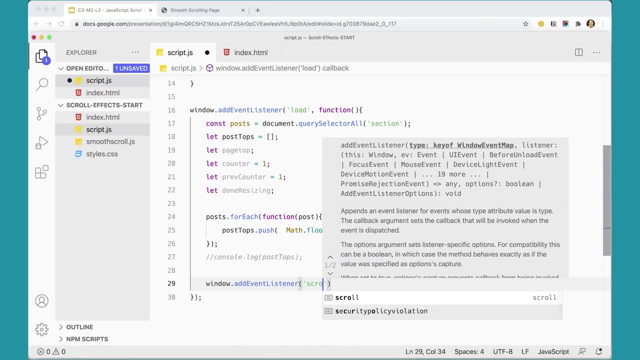 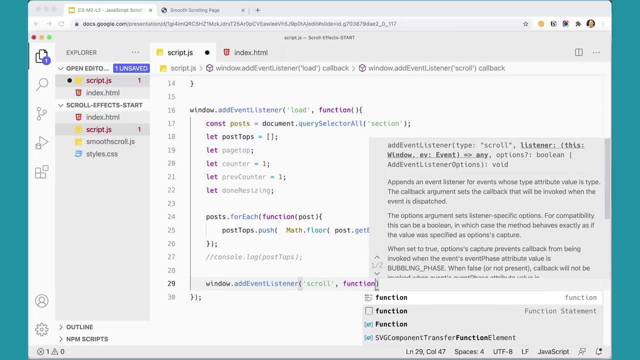 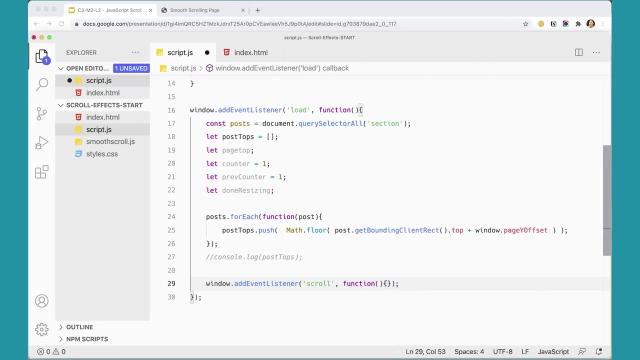 for capturing scroll effects. So again, I'm going to attach it to the window- windowaddEventListener- And we're listening for scroll scrollEvent, And then we're going to run a function Like so And all of our stuff will go inside of here. 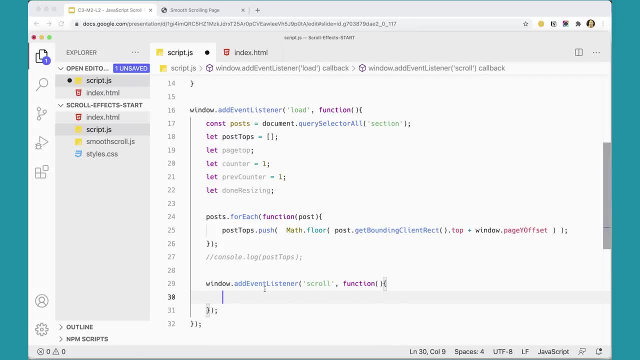 Now this looks very similar to the jQuery version of the scroll event. In jQuery, we did it like this: We used the jQuery object to grab our window And then we used the on method to capture, scroll And then run a function. 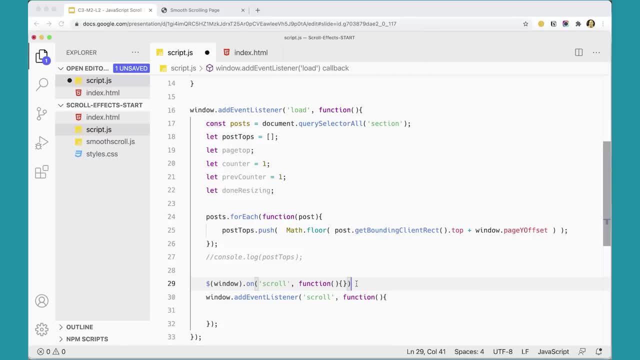 So again, it looks very similar, but just slightly different. And yeah, the jQuery version is a few characters shorter, So that makes learning this stuff a little bit easier. I think in jQuery, But the plain JavaScript syntax is not that much longer. 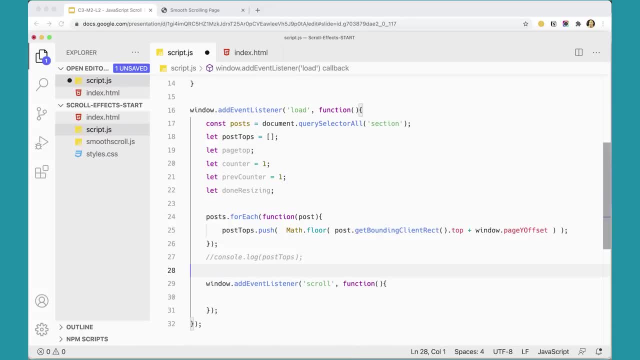 And you don't have to download the entire jQuery library to use it or force your users to download the entire jQuery library to use it. So that's kind of nice, All right. So then we're going to put into this variable pageTop. 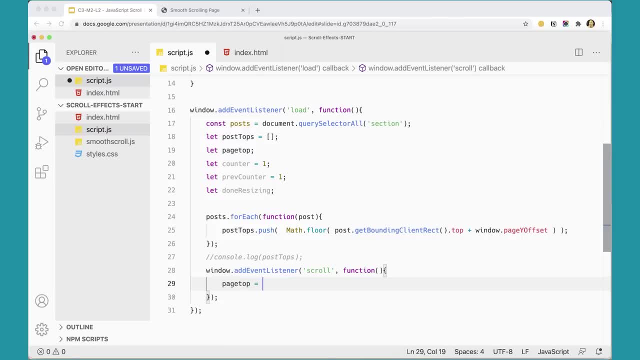 pageTop is going to equal this thing, windowPageYOffset. And again, what that does is windowPageYOffset tracks how far up off the top of the window our page has scrolled. So I can consolelog pageTop And we should be seeing. 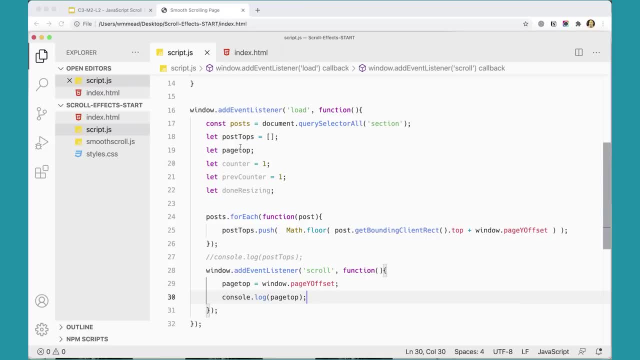 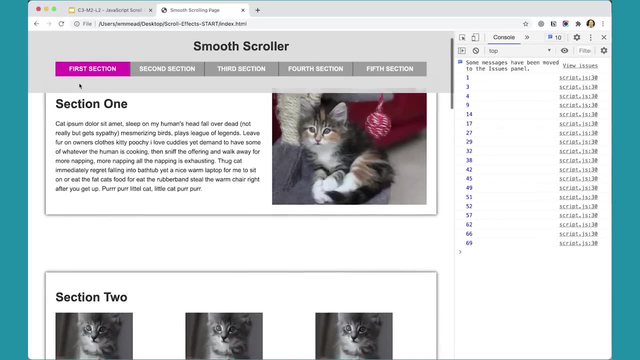 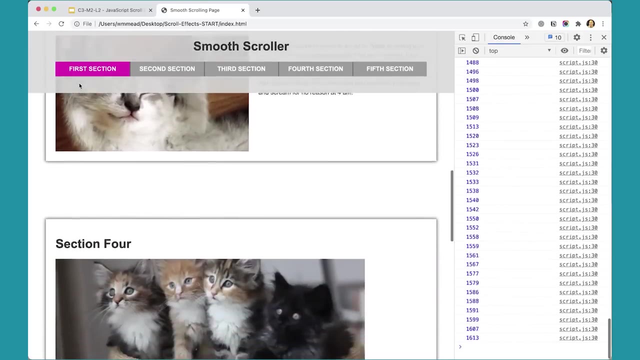 those pixels change as we scroll down the page. Let's test that and see. So I come back here and refresh my page. Now, as I scroll down the page, you can see those pixels are going up And again as before with the jQuery version. 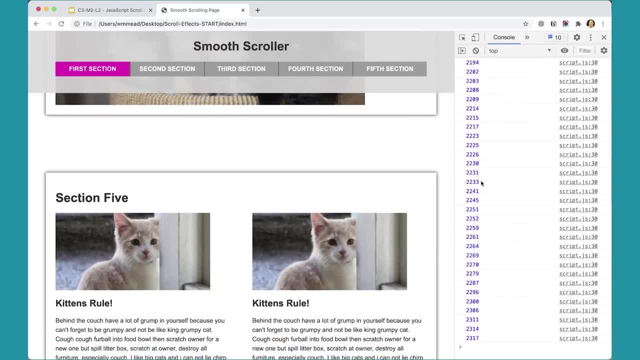 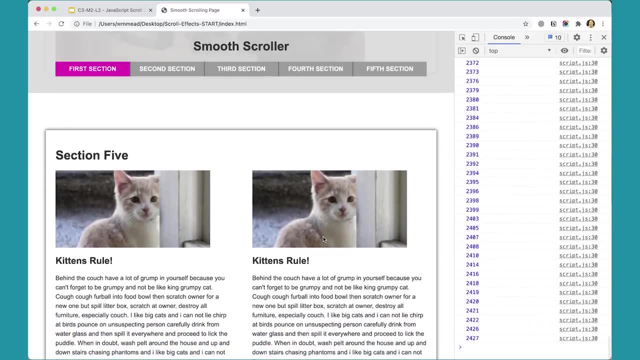 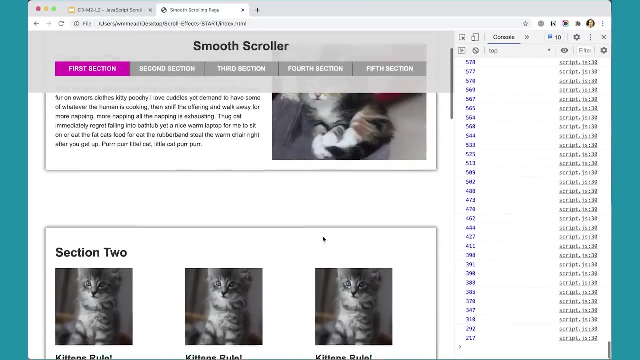 we're capturing every little bit that scrolls, But we're not necessarily capturing every single pixel. The slower we scroll, the more pixels we'll capture, But the faster we scroll, the fewer pixels we'll capture. But that event is firing every time we scroll a little bit. 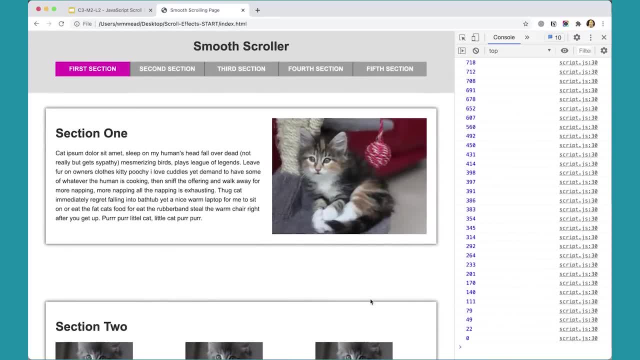 We get up to the top of the page, we should be getting a zero. When we get down to the bottom of the page, we should be getting a number that represents the full height of the entire window. That's working great And really what I want to do. 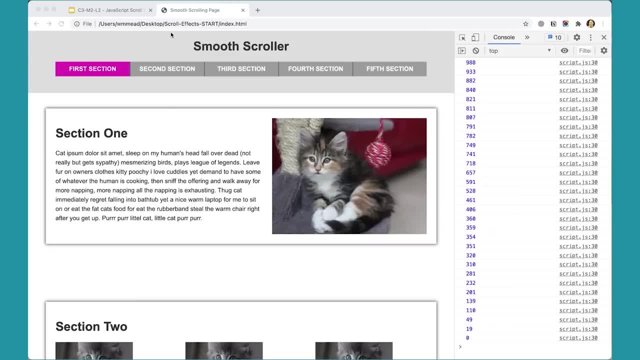 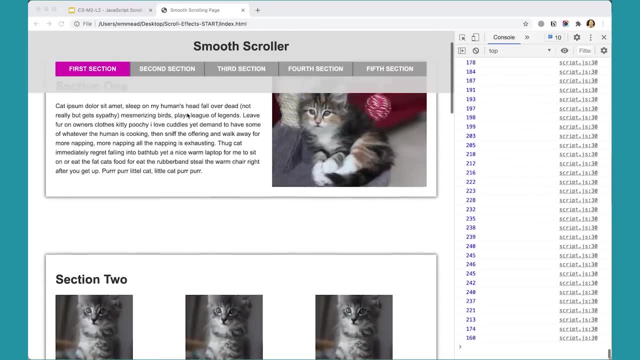 is. I want to track not the very top of the window, but the start of this first thing, or maybe a little bit down from it. I want to push down a little bit from there. So, really, what I want to do is I want to come back. 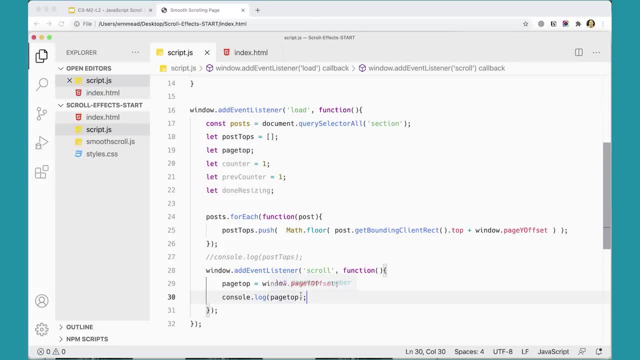 and add 250 to this. I did 210 in the other one, but I'm going to do 250 here, So I think it's a little bit better. So I'm going to add 250 there And it's worth noting. 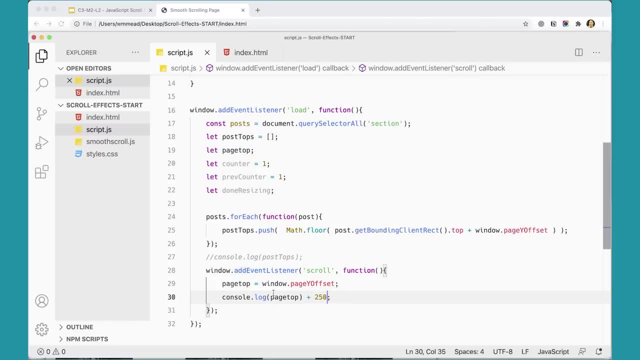 that the strategy for this script is exactly the same as what we did for the jQuery script. When this number, the page top number, is greater than the number of the second section for post tops, where that one starts, then we must be viewing: 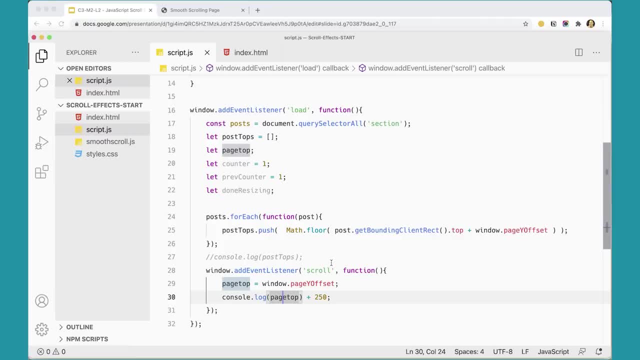 that second section on the screen, And if it's greater than the number for the top of the third section, then we must be viewing that section on the screen, and so on. So that strategy is exactly the same And, as before, you can either be scrolling. 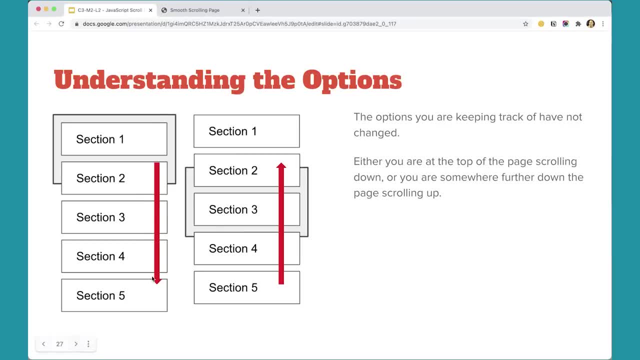 down the page, starting at the top or going down, or you could be somewhere in the middle of the page and scrolling up. Those are really your only two options, because this page doesn't scroll left and right, It only scrolls up and down. 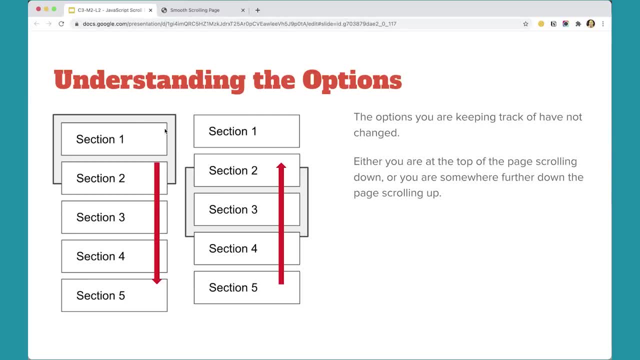 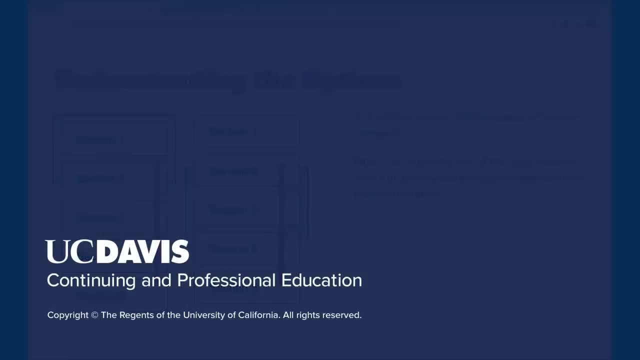 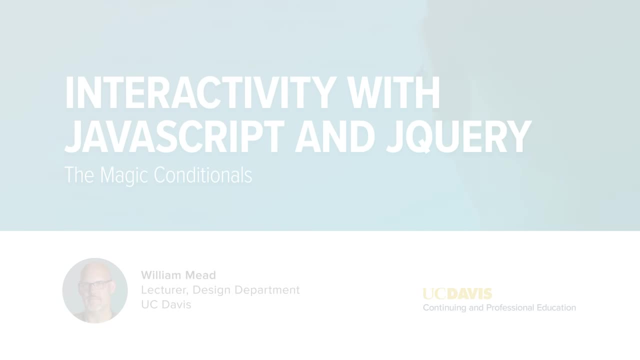 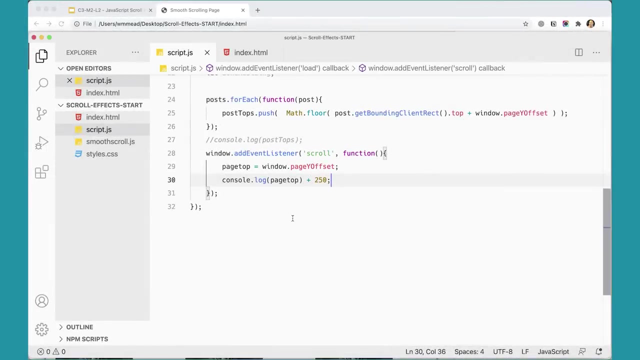 So those are your only two options. So those are the two conditions that we need to watch out for while we're handling our scroll effect. To handle those two situations of scrolling up and scrolling down, I need an if and an else. if, just as I did. 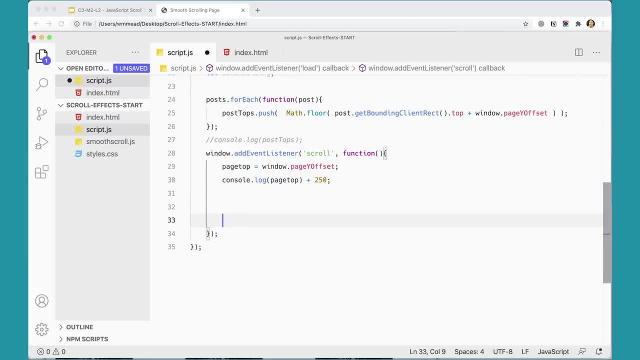 in the jQuery version And I'm going to pick this one up here. You're going to have to type it, but I'm going to paste it in here because it's actually exactly the same as what we had in the previous script And, in fact, 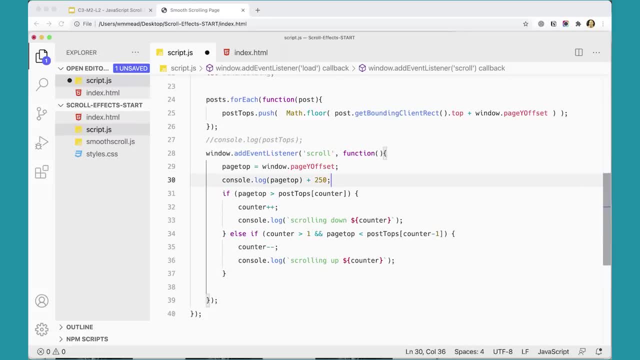 I don't think it's different, really even at all. I'm going to comment out this console log call there. We don't really need that now, But here I'm seeing if page top is greater than the post tops counter, So the counter starts at one. 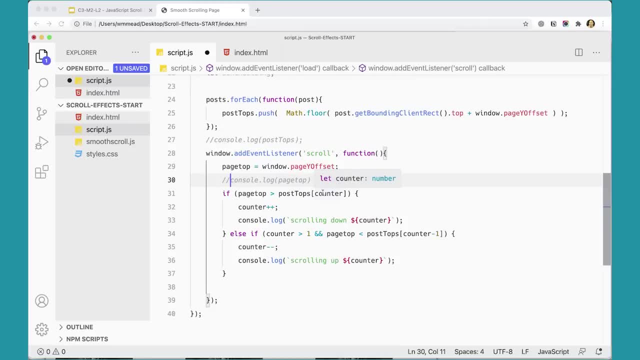 So if it's greater than the first element inside post tops, the counter is going to get incremented. So if we're on the first section and we go into the second section, this counter would be one, And so now we're in that second section. 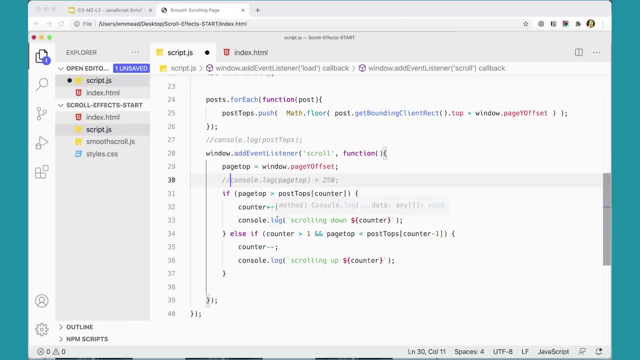 So then we should increment the counter, And we must be scrolling down, And then when we go into the third section we'll increment the counter again, and so on and so forth, as we get down to the bottom of the page. Then the else if 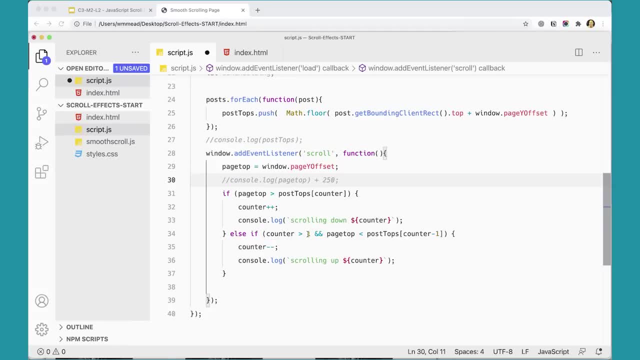 we're going to check to see if the counter is greater than one- not greater than zero this time, but greater than one. Is it greater than one? Because one is our first section, And if page top is less than post tops, counter minus one. 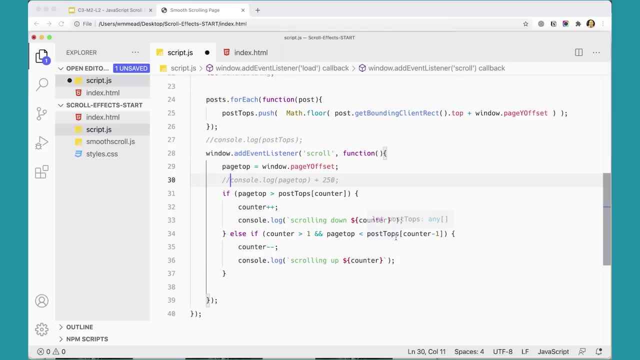 So if it's less than one, then we must be scrolling up if both of these are true, in which case we'll decrement the counter. All right, let's give this a try. This should be showing us in our console over here. 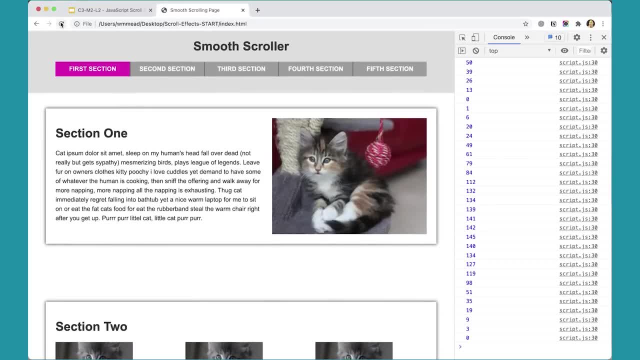 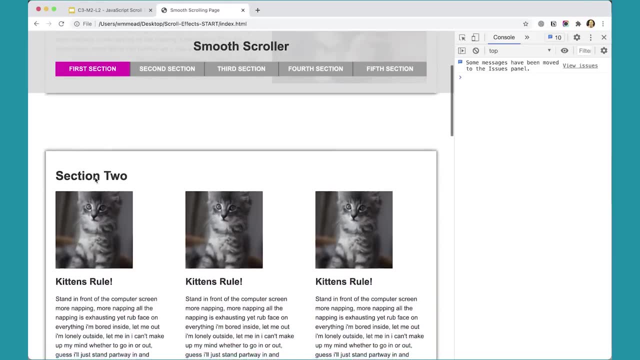 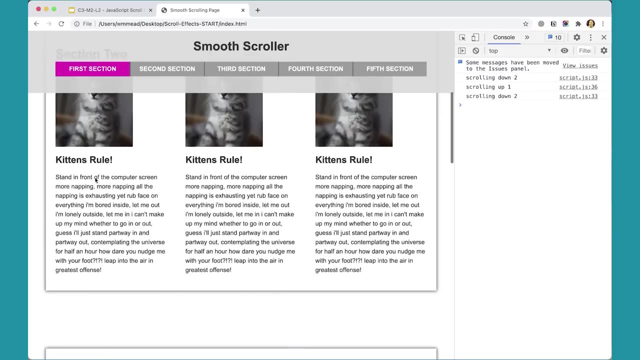 We come back, scroll up to the top of the page, click refresh and then scroll down the page. When I get to that second section, that second section, it's 250 pixels from the top of the screen. It now says scrolling down two. 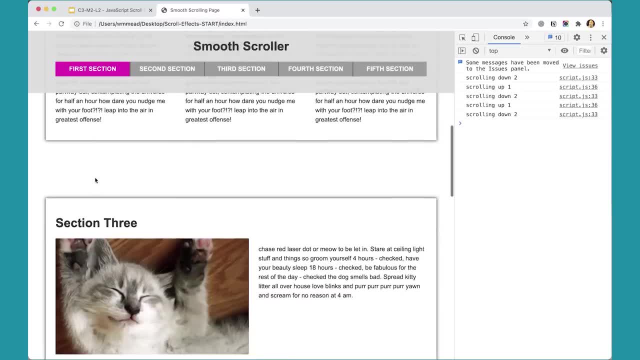 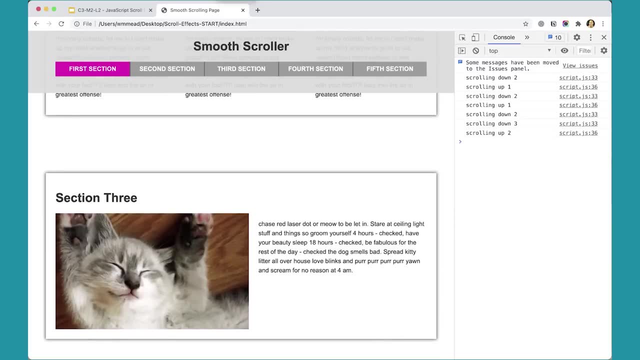 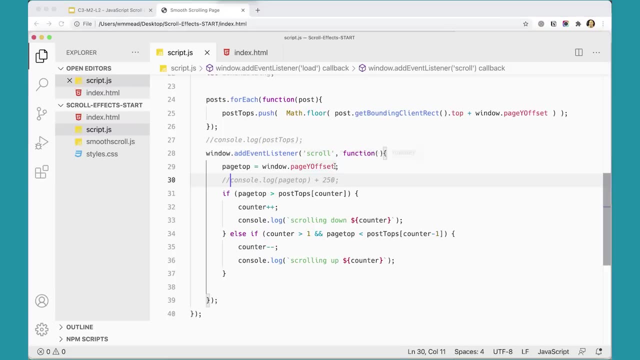 And it didn't do the 250 pixels, though did it? It should be doing it there. I see what I did wrong Over here. I put the plus 250 in the wrong place. It should be here: Plus 250.. 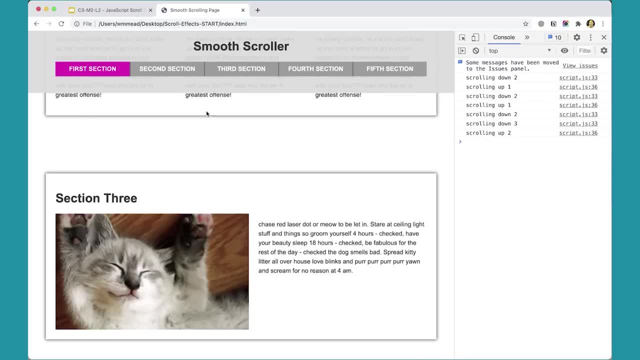 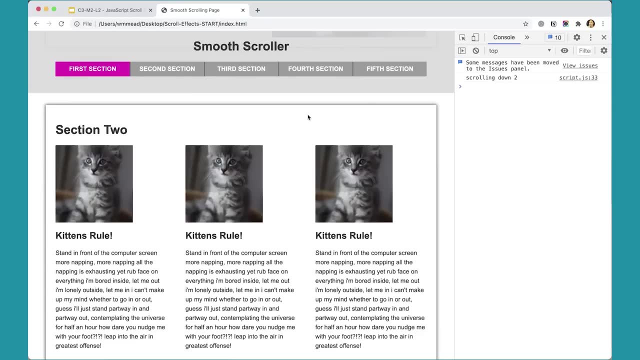 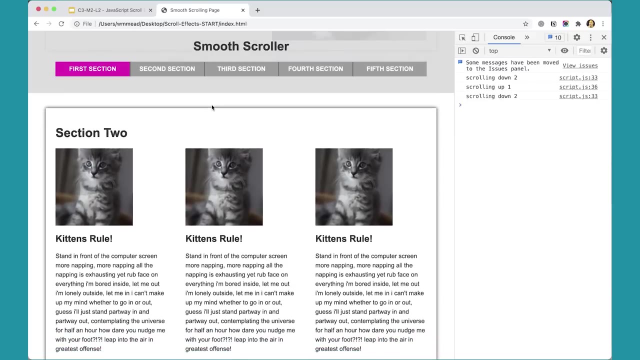 There we go. Let's try that. Scroll up to the top of the page. There we go. Now, when I get to section two, scrolling down two, when that is 250 pixels from the top of the page, it hits it and says: 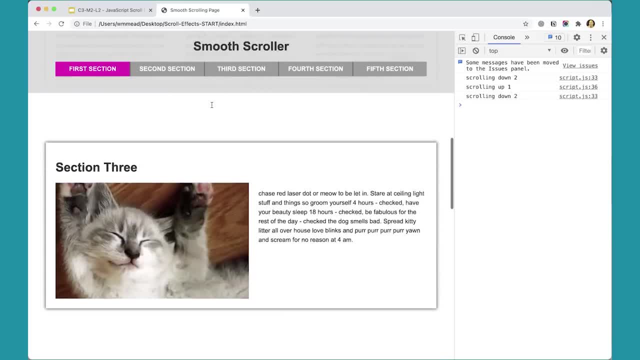 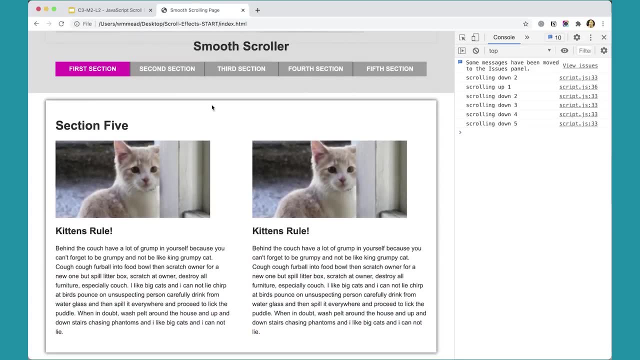 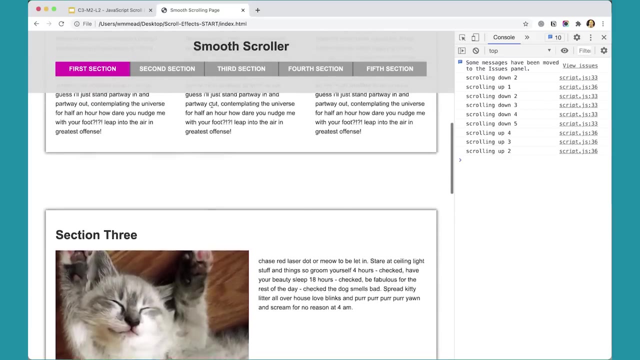 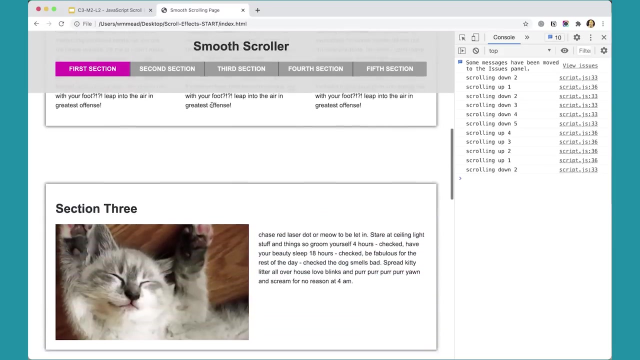 okay, we must be looking at section two, And this one gets to 250.. We've got three, four, five, and then when we go up we get four, three, two, one. So that's working great. So I can tell this thing is firing. 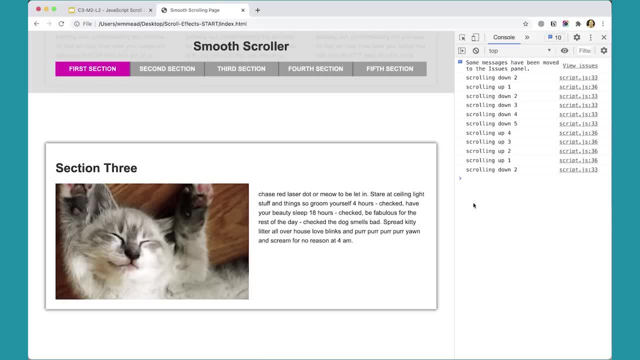 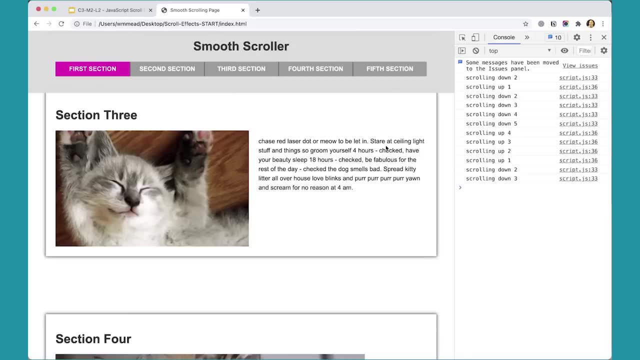 I'm not getting calls for every single little smidgen that I scroll. I'm only getting calls when that section comes into the page, And that's the beauty of this script. I think it's really wonderful. I love it Okay. 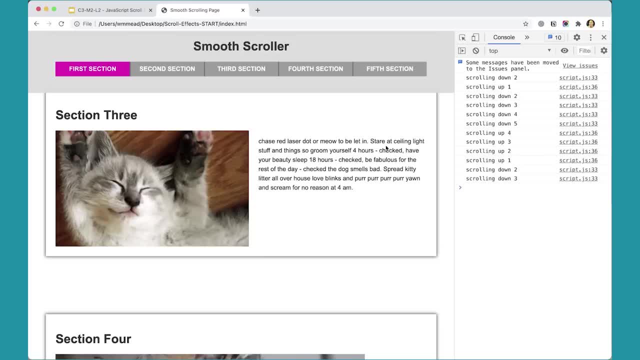 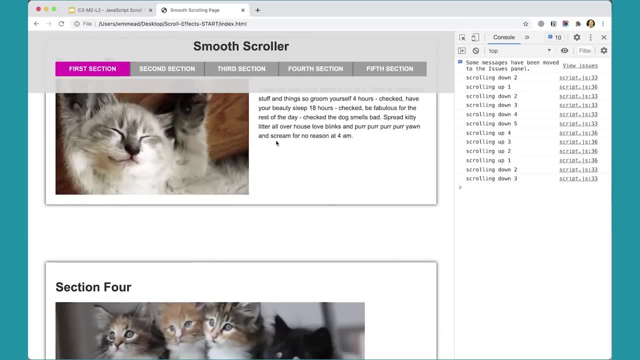 And that's what we were able to do with the jQuery version as well, And that's what makes this script very powerful, because only when those things happen we're going to make other things happen on the page, not for every single pixel that we scroll. 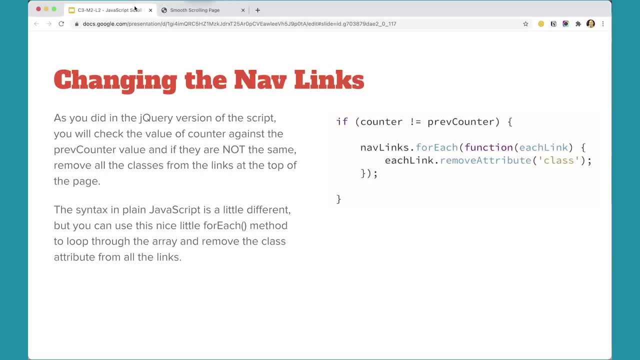 Just as before, we want to see if the counter is not the same as the previous counter, because if it isn't, then we've moved into a new section And the first thing we want to do is remove all of the classes from those links at the top of the page. 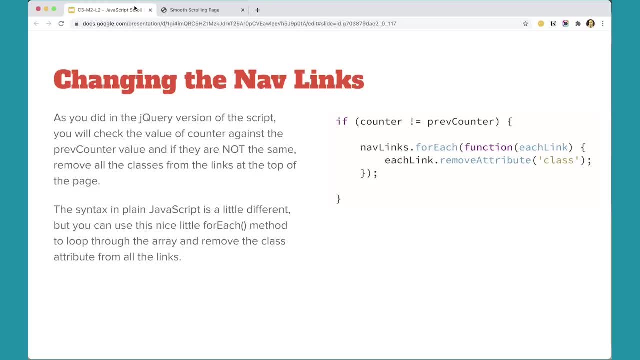 which is that class selected. that should be on one of them, But we want to make sure it isn't on any of them. We'll remove that class attribute from everything, just to be clear that everything has no class on it up there. So let's go ahead. 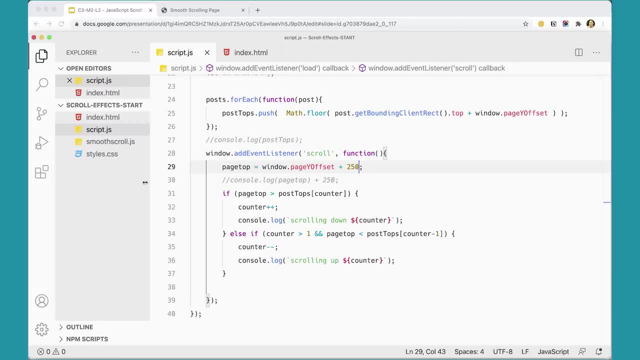 and add this if statement over here. So down here I'm going to add an if, If counter is not the same as previous counter. if they're not the same, then again I'm going to use my forEach And I already have up here. 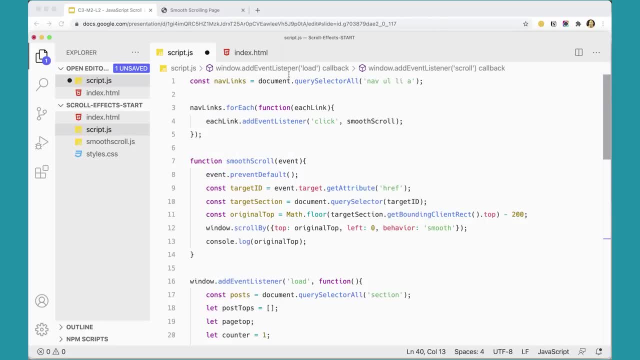 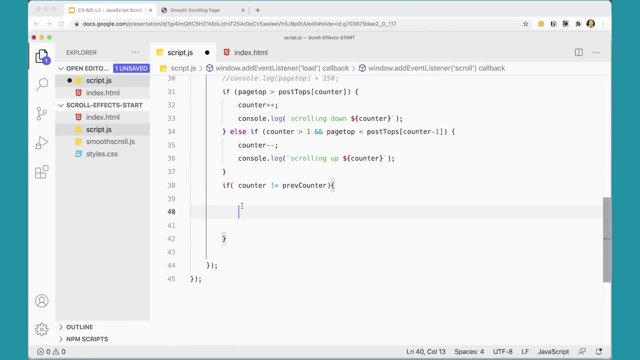 at the top of the page. I already have navlinks gathering all these, So we've already got this variable, So we can just use it again. And, just like before, I'm going to just do navlinksforEach function. curly braces: each link. 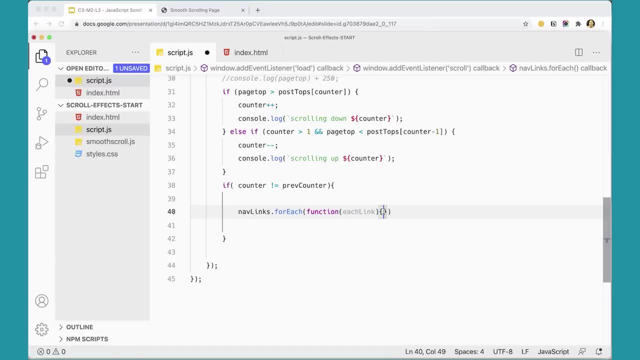 It's going to go through each link of navlinks And what is it going to do here? We're going to say, okay, each link dot, remove attribute This one. here, Which attribute are we removing Class? So that'll remove the class attribute. 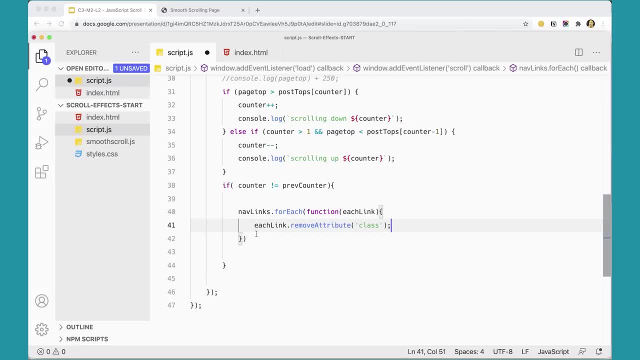 from each of those Great. We'll stop this video here, but in the next one we'll put the correct, the correct item on the correct link, the correct class on the correct link. We'll put the selected class in the link that was clicked. 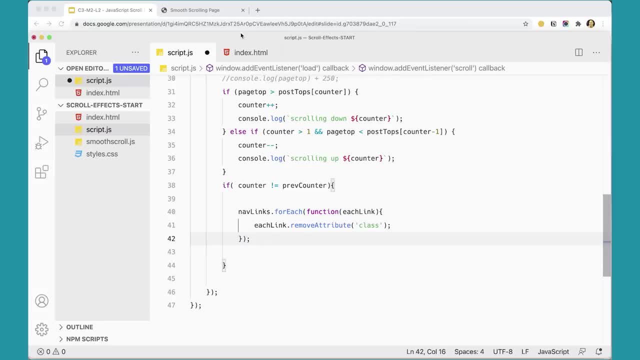 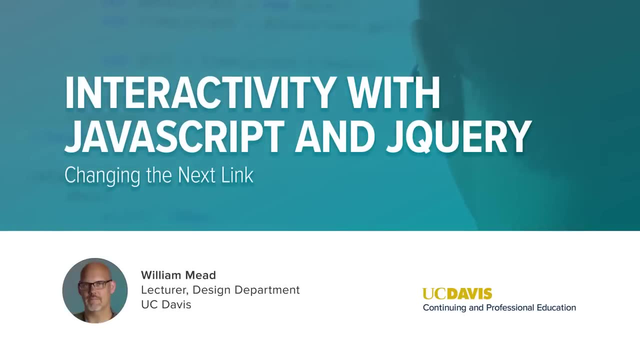 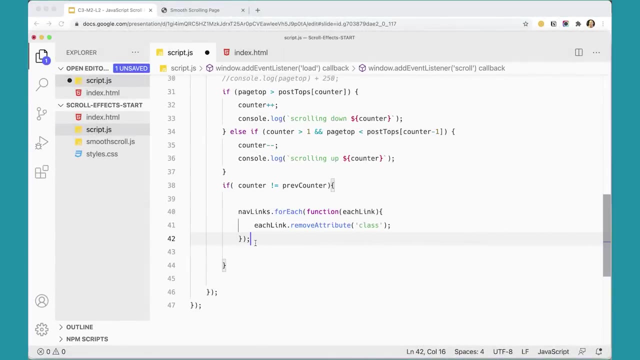 so that it can get highlighted properly. Put a semicolon there before we go. We took the class attribute off of all the links. Now we need to add it to the correct link, So I'm going to add a variable const this link. 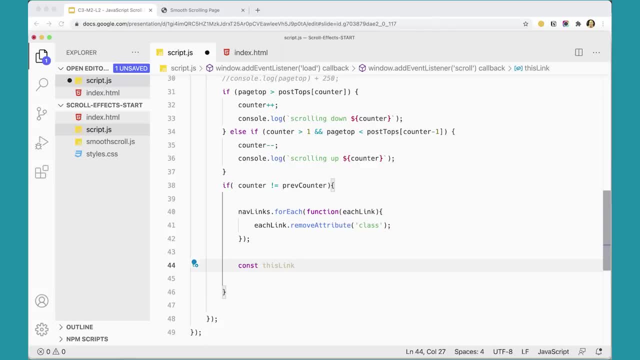 I want to add it to the link that I clicked on And I'm going to use. I'm going to use, I'm going to get the correct link here by using the query selector. So I'm going to say document dot query selector. 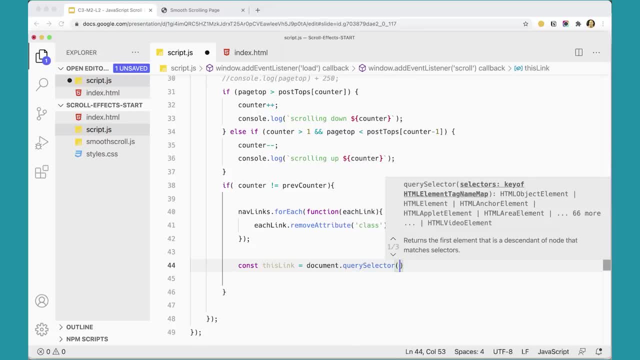 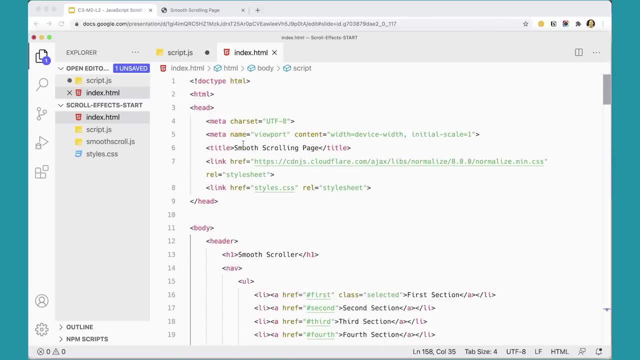 query selector. And this is a little tricky, this query selector. What we're going to use is nav ul li a, But we want li, colon nth- child parentheses, Because over here in our HTML, remember, we want to get if we clicked on this one. 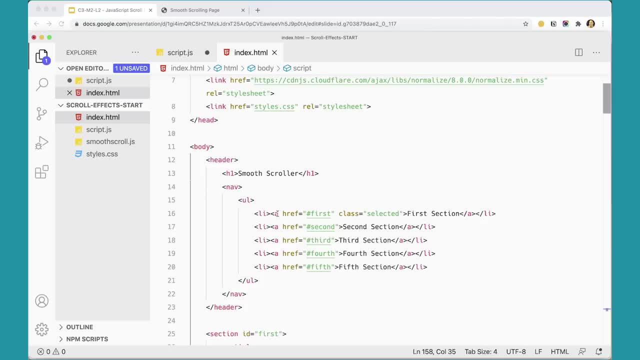 we want to get the first list item's anchor tag or the second list item's anchor tag or the third list item's anchor tag. Remember, the list items are all siblings. The anchor tags are cousins. There's only one anchor tag. 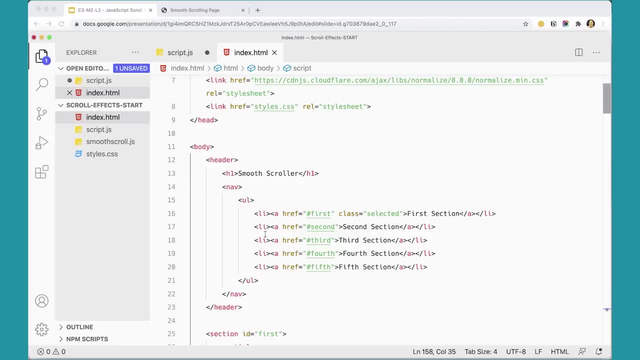 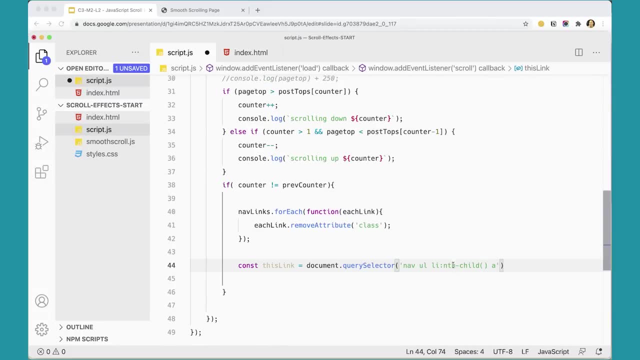 in each list item. But the list items are all siblings. So there's, this is the first, one, second, one, third, one, fourth, one fifth one. So over here I want to get nav ul li, nth child, And if I were to put in a one, 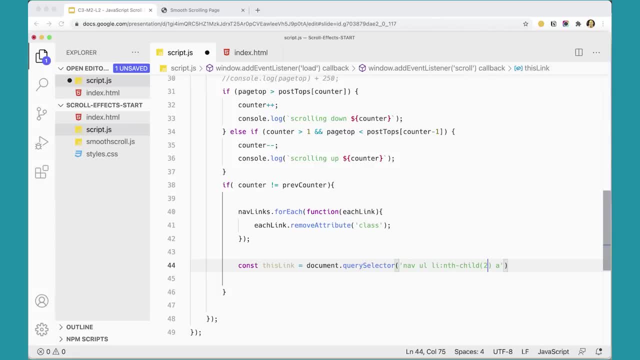 that would get the first link, A two would get the second link, A three would get the third link, And so on. So this is why we're using one, two, three, four and five for our counters, instead of zero. one, two, three. 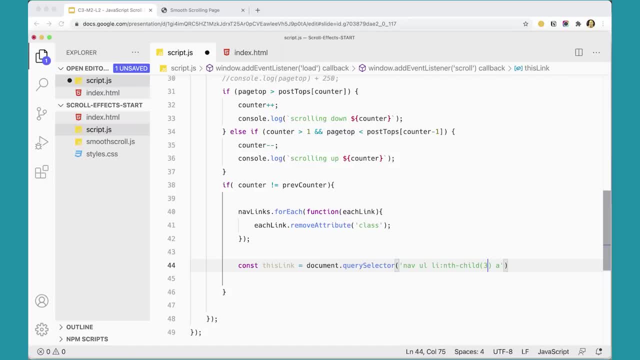 and four in this script. In the jQuery script, we use the eq method to find the first, second, third and fourth link, But that's zero indexed. So the first one in that one is zero, whereas the first one in this one is one. 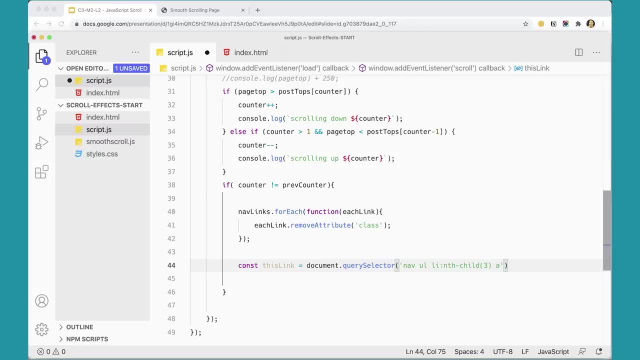 So that's why our counter's a little bit different in the script. But we could have probably used the nth child method in the jQuery version and had it be the same now that I think about it. And that would be another way Because, remember, in jQuery 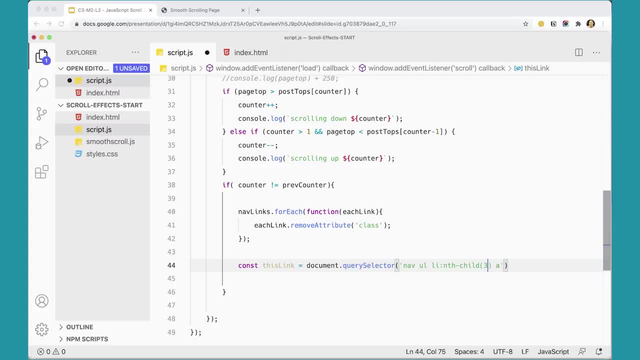 there's about a hundred ways of getting to each element on the page, So we could have done it this way as well there, But what I want to put in there is my. what I want to do is: I want to change this, so I'm using my. 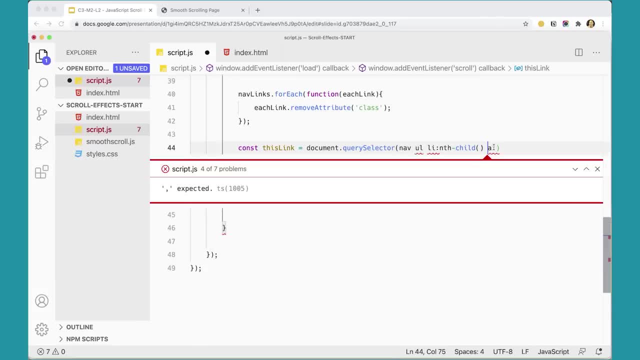 not my up and down quotes, Oops, Yeah, yeah, I know it's a problem. I want to use my tick marks so that in here I can pass in dollar sign curly brace counter And that will put the correct counter. that will get me the correct link there. 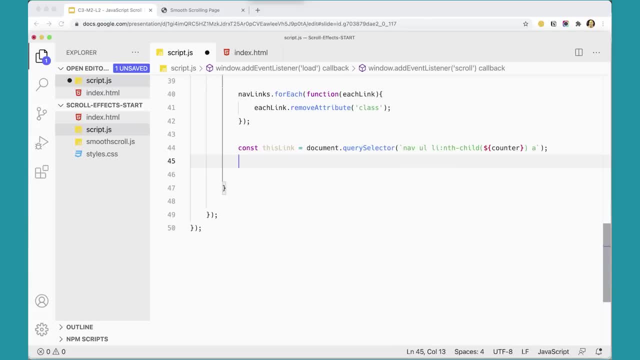 From there. it's simple. I can just now. I can use this link: dot. class name is selected. Make sure you spell selected right. And then of course we want to say prev. counter is now assigned the same value as counter. Because now we're ready. 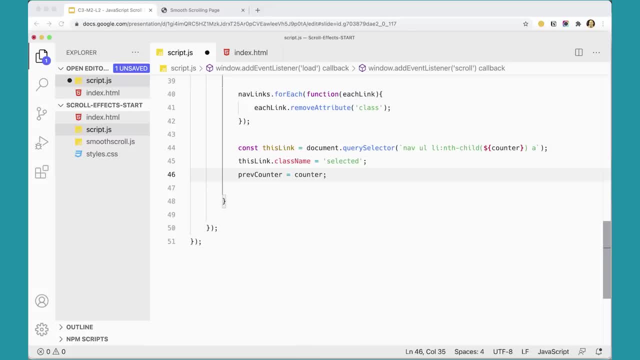 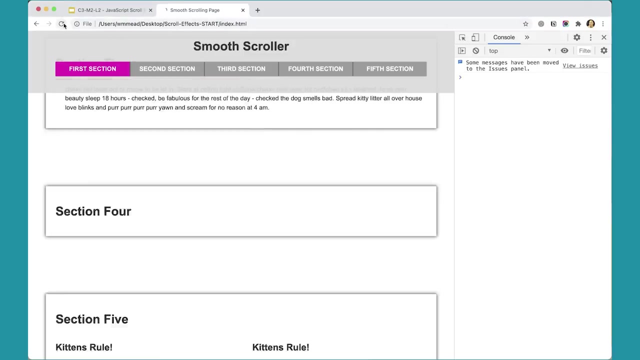 to go into the next, the next section. So if I save that and test it, assuming I did it, all right, it should work. Let's see Refresh the page. Start up here at the top. We'll get that. It's already working. 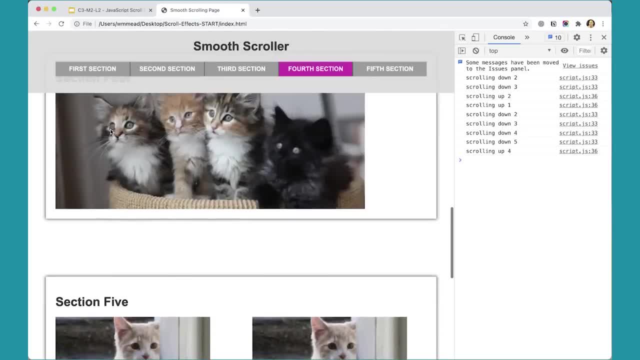 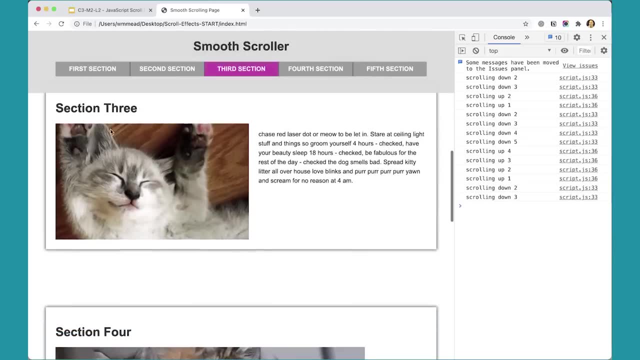 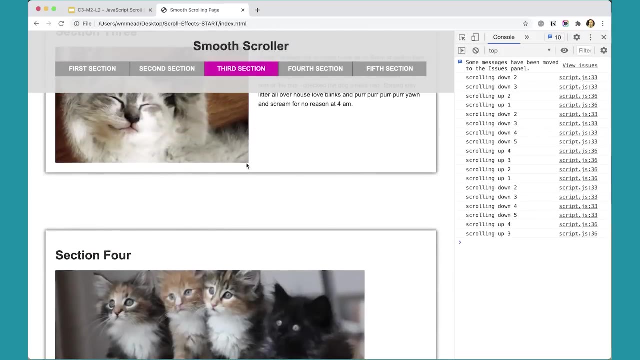 Second, third, fourth, fifth section. So that's working perfectly fine. It's nice and smooth because the animation is happening with in the CSS And the JavaScript is super efficient because it's only calling these as you move into these sections. 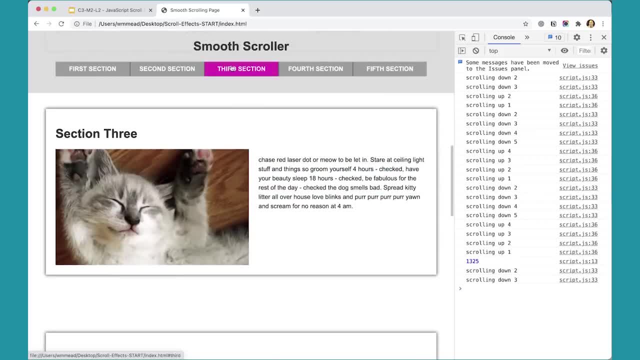 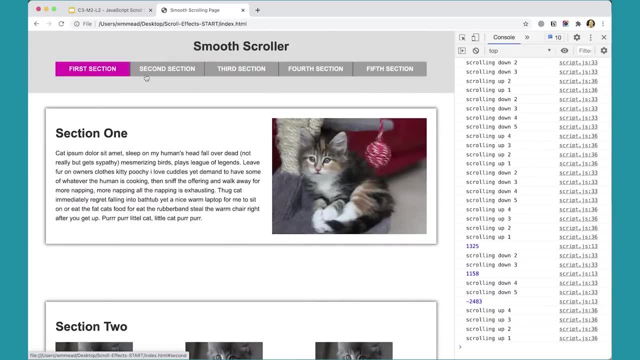 And not only that, but when you click on these it'll actually highlight the correct section as you're going to, and even sort of highlight in between. It's that fast, So that's working really great. I'm really pleased with the way that works. 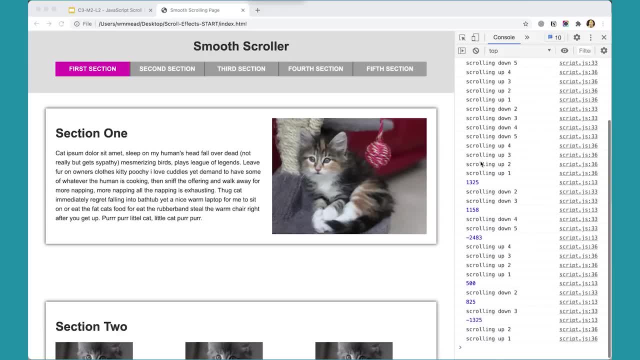 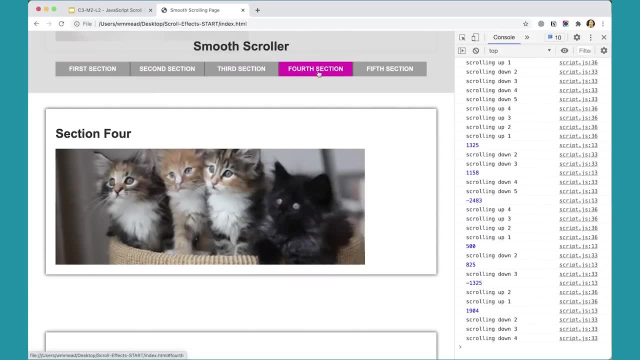 Over here in my console log I can see where I'm scrolling up and scrolling down, And these numbers must be coming in. when I'm clicking on one of these links I must have left a console log open in that script as well, So we could go over. 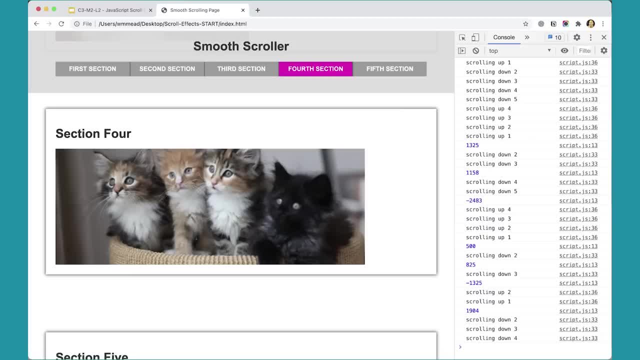 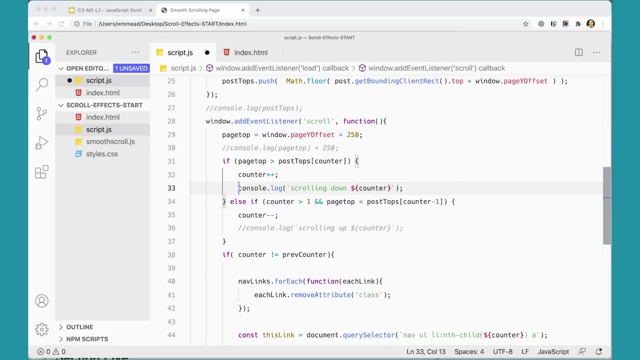 and kind of clear out these console logs. We don't really need them all. They're kind of handy to have while we're making the script, but we don't really need this one or this one. We're up here. I must have one up here somewhere as well. 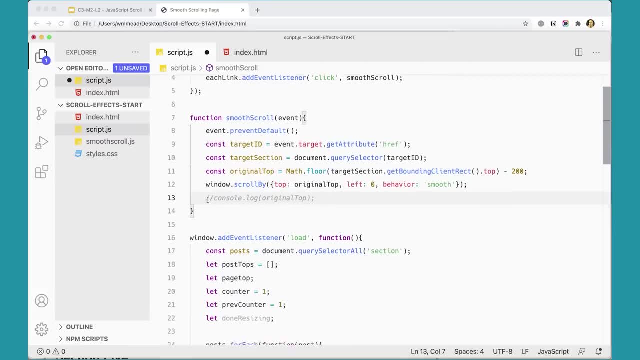 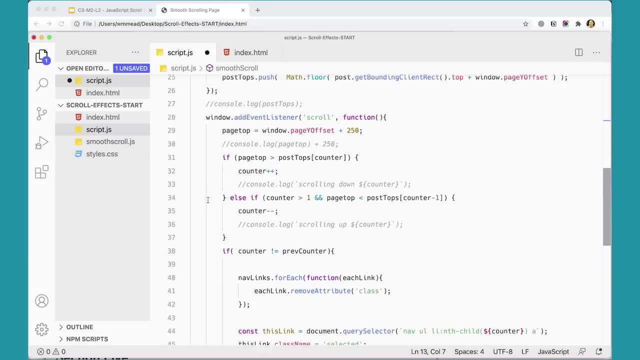 Here it is original top, So I don't need those, Or you could just delete them all together And that's great, And this script is working. The last thing that we need to do is take care of this situation. There's edge cases of what happens. 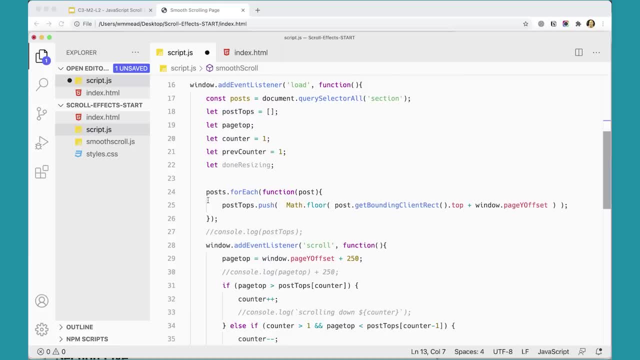 if somebody is resizing the window, or if they refresh the page while you're scrolled down the page, And so we'll take care of that in the next video, And then we're done with this script And you'll have two versions of it. 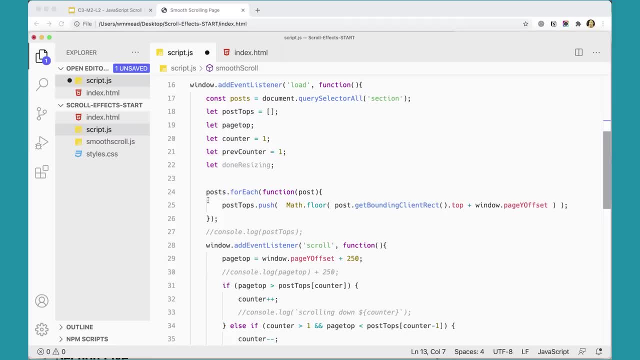 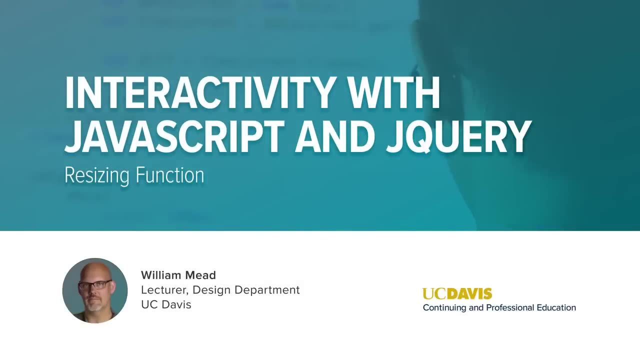 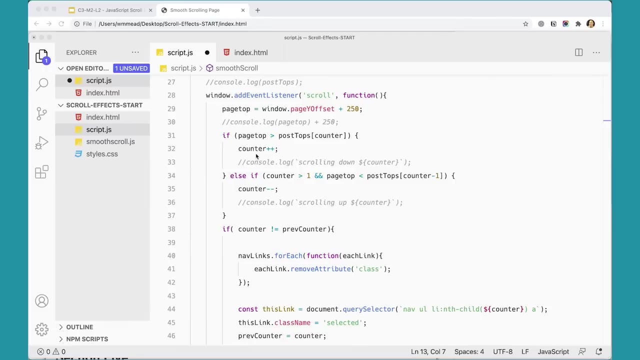 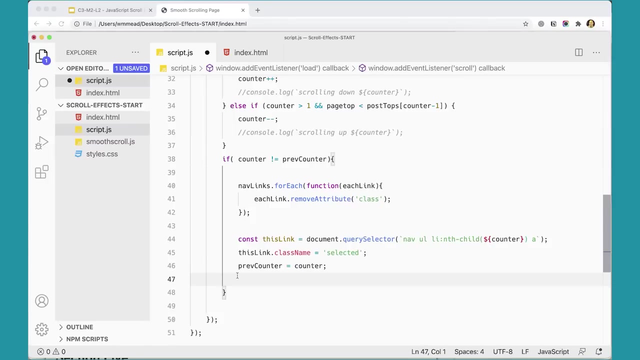 one that works with jQuery and one that works with plain vanilla JavaScript. Just as we did before, I want to add an event listener that captures when I'm resizing my window. So over here, I'm just going to get rid of a little bit of spacing in here. 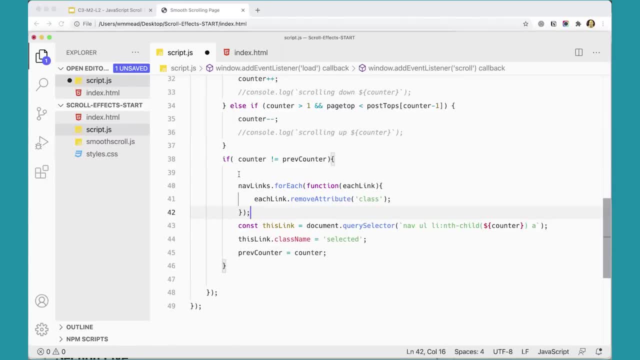 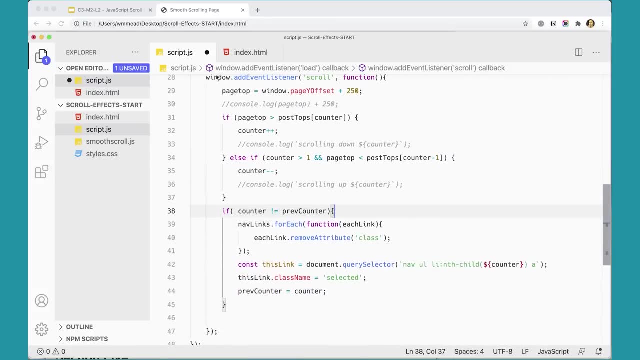 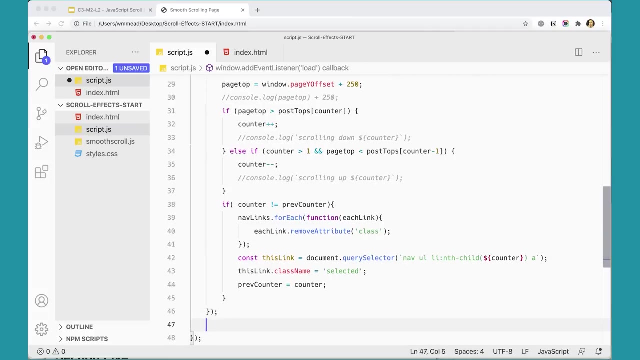 just because I want to be able to see everything here, All right. So I want to add this event listener after the event listener for my scroll function here. So I want to add it after that, but before my event listener for when the window loads. 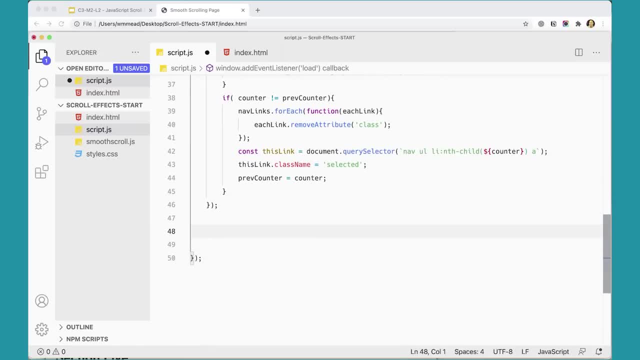 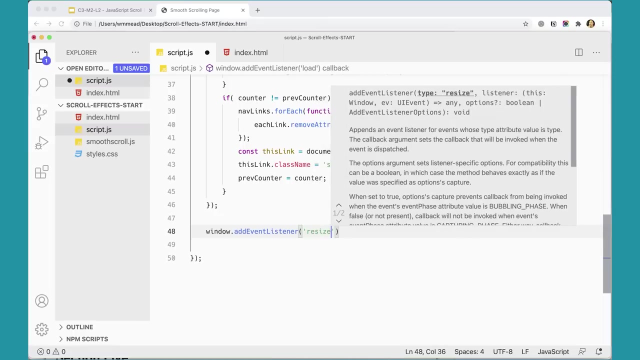 So I want to add it in here. So make sure you're putting it in the right place, because that's really important. And here I'm going to just do windowaddEventListener and I'm going to look for a resize event. I'm going to type a function. 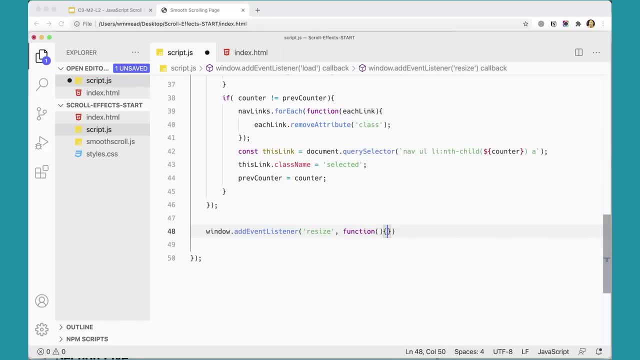 That's going to run when the window resizes semicolon, And we will put stuff in here Now. remember when we were doing jQuery. we used our jQuery object to get the window and we used the on method to then capture the resize event. 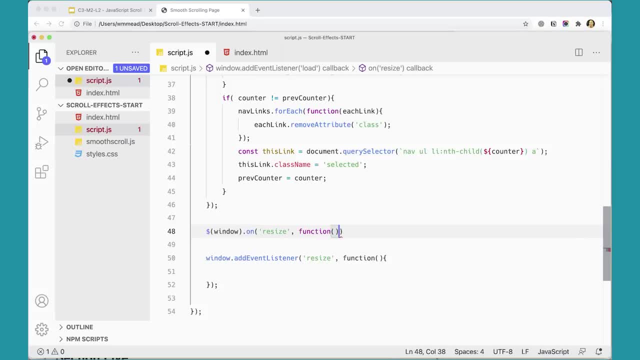 and run a function. That's how we did it with jQuery. So here the syntax is slightly different, but not that different. We're just adding an event listener to the window and resizing it for when we resize, So it's not that different. 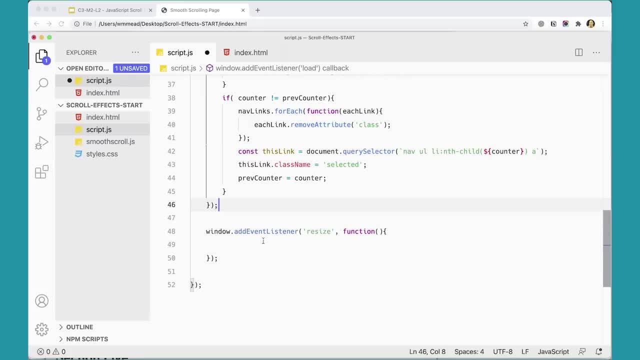 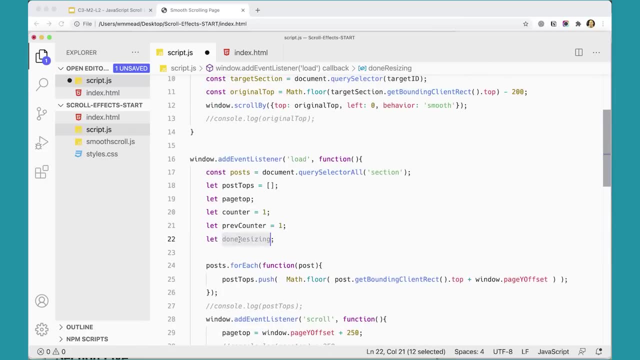 It's a little bit different And the jQuery is a little bit shorter, but that's okay. Once we're in here, what we're going to do is we're going to use this variable that we've left up here, doneResizing. 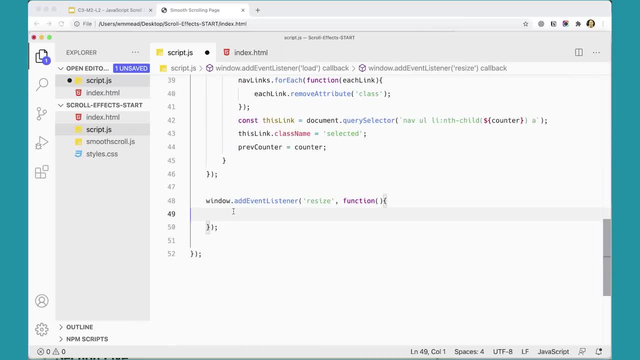 And we're going to say doneResizing dot equals. No, I'm doing this wrong. I need to do clearTimeout, clearTimeout, doneResizing, And then I need my doneResizing equals setTimeout. That's what it looks like: setTimeout And setTimeout runs a function. 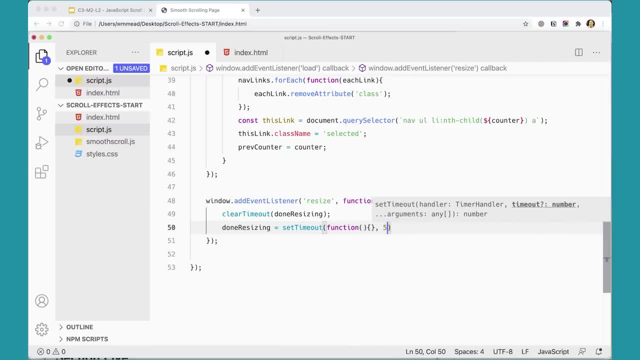 after comma, a certain period of time: 500.. So this is exactly the same as what we had before And basically what's going to happen is this is going to capture while we're resizing, but clearTimeout is going to keep this thing from actually doing anything. 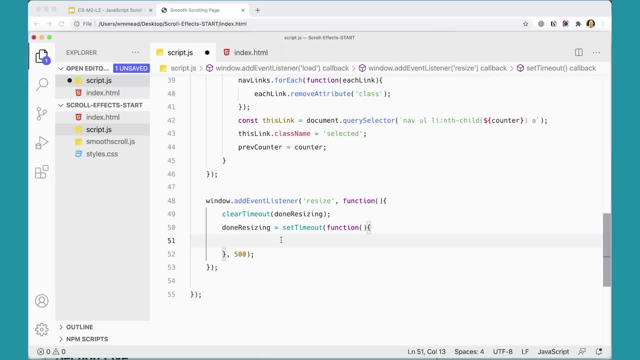 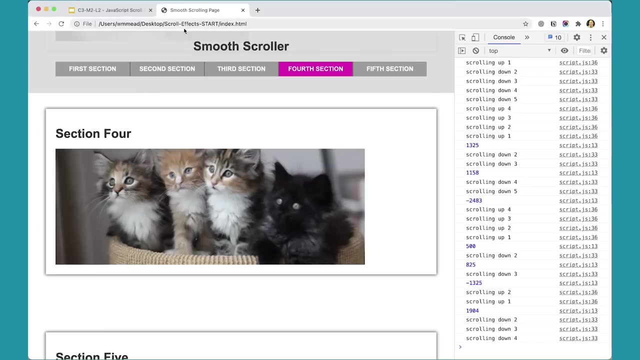 until we're done resizing. So we only want to capture this when we're done actually resizing the window, consolelog doneResizing, Which will happen 500, half a second after we're done actually resizing the window. So let's just test that really quickly over here. 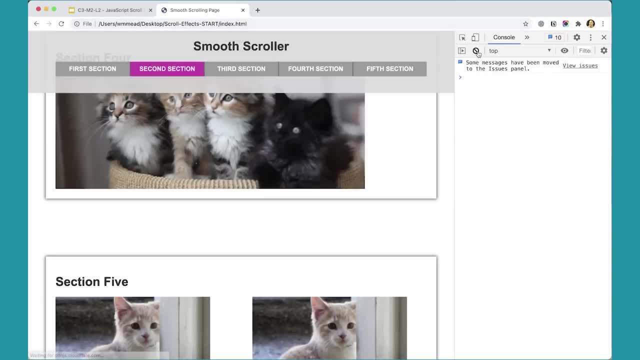 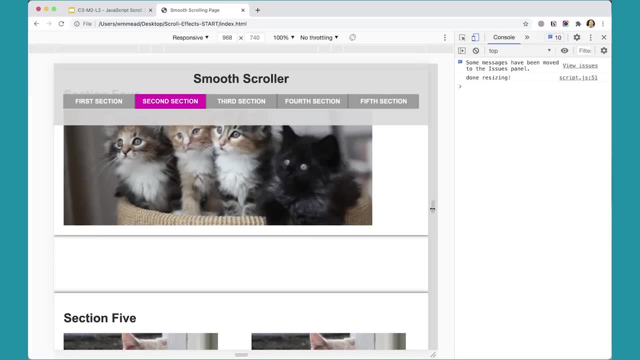 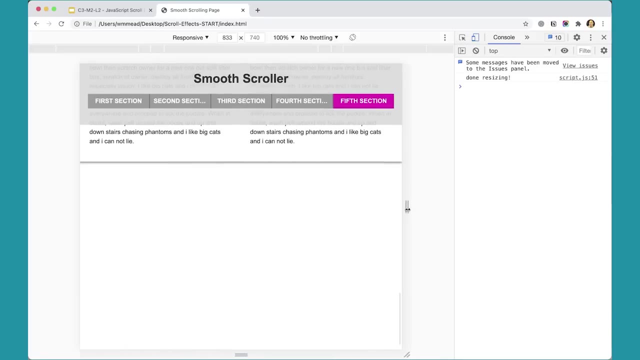 I'm going to refresh the page And I'm going to click this button here to get into resize mode And then I can resize this window up and down and sideways and do all this stuff, But it's not going to actually do anything until I let go and stop resizing. 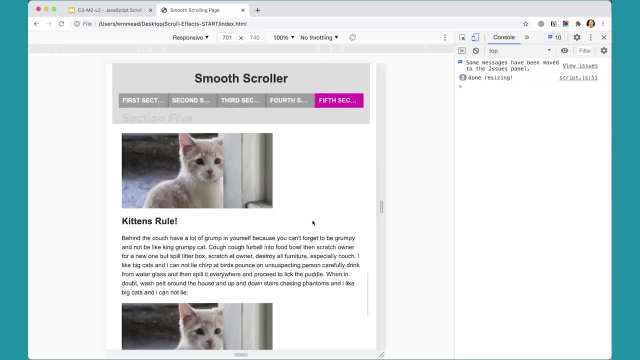 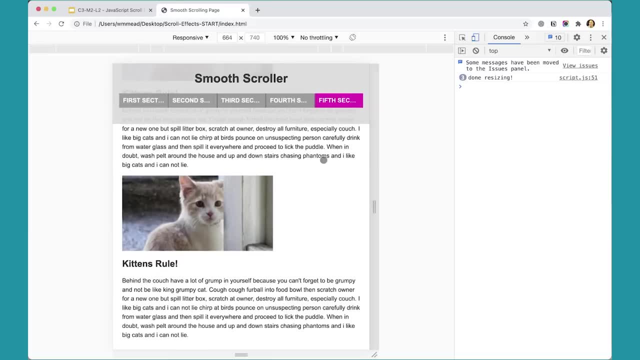 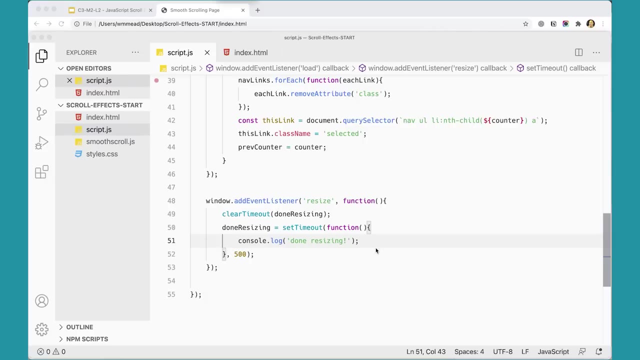 In that case it'll say doneResizing at the end of that: doneResizing, Okay, great. So what am I going to put inside there? that's going to run when I'm done resizing. I'm going to add my function. 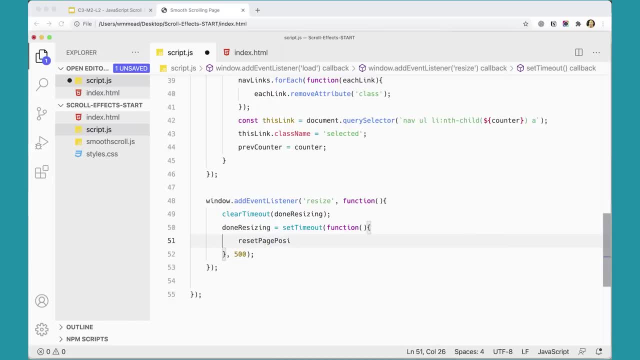 resetPagePosition- I think that's what I called it. That's the same function we had before in the jQuery version. So I'm going to come down here and add a function function: resetPagePosition. parentheses, curly braces And we will go on from there. 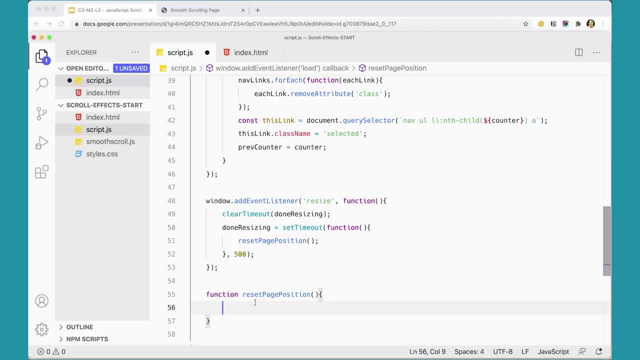 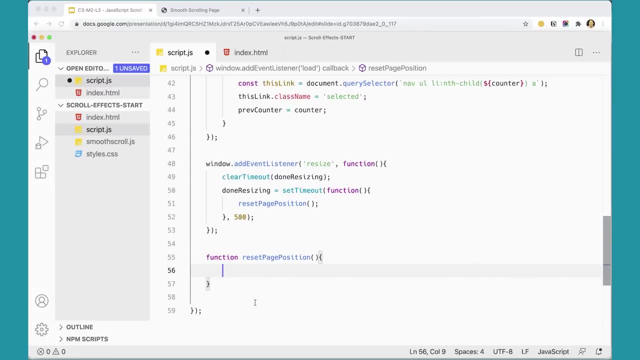 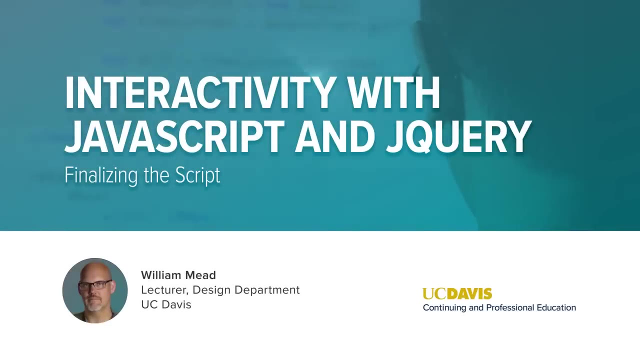 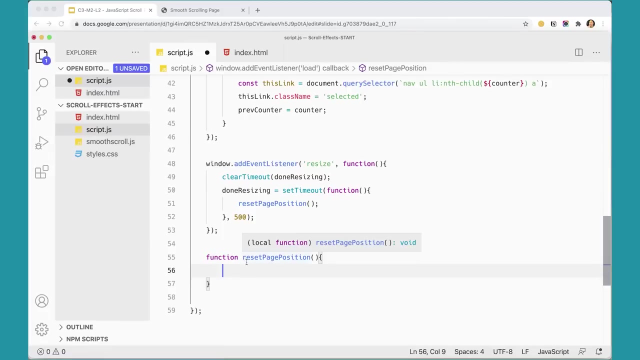 and we'll build that up in the next video to kind of finish this script off. But this is really all exactly the same as what we did for the jQuery version. We're down to the end of this lesson and we just need to fill out this. 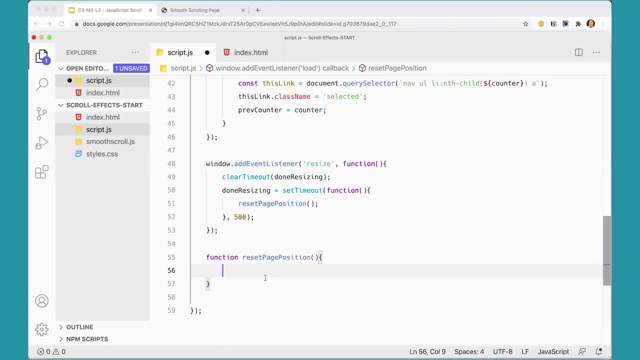 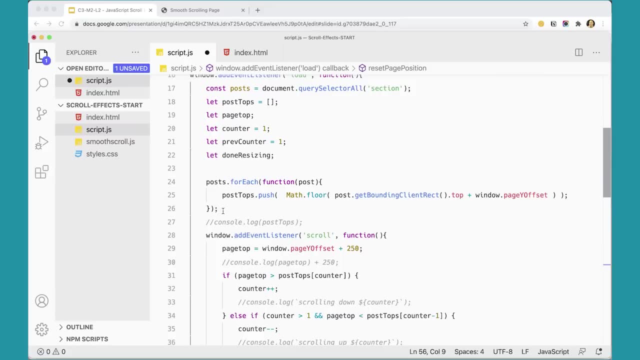 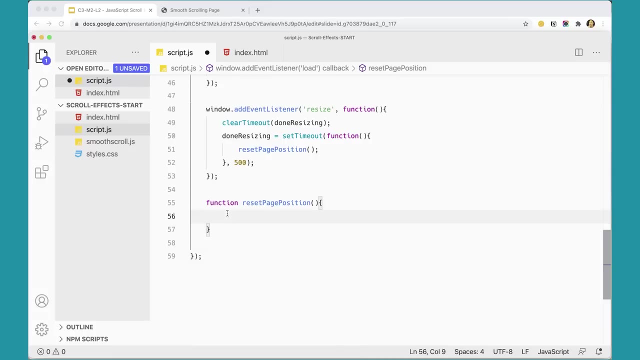 resetPagePosition function here, And we're going to start by coming up here and basically just stealing this thing here and sticking it in here. I also want to have make sure postTops gets reassigned- an empty array- just to be absolutely certain that that thing. 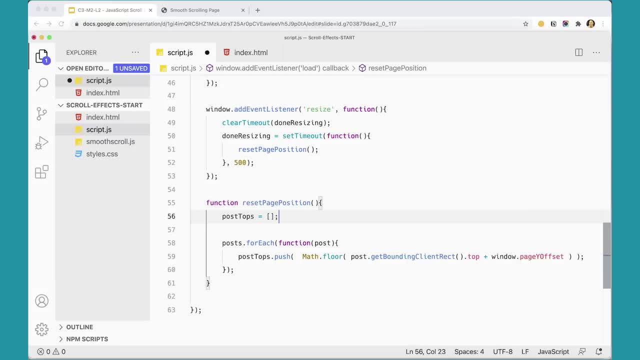 is empty, And then I'm going to go through each of my posts and push into there the top of that postTop. So that makes sure that, again, if I'm resizing my window and recapturing where the tops of each of those sections is, 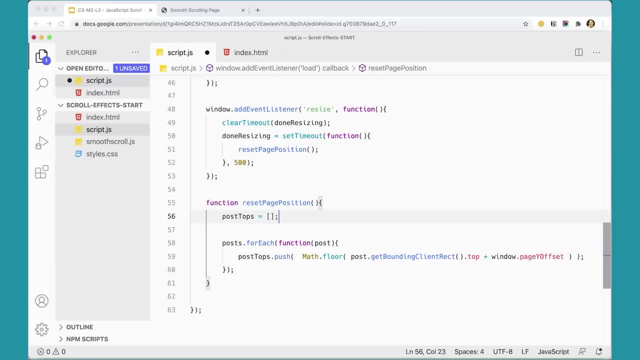 because they may have changed based on how wide the window is. once I've finished resizing it, The next thing I want to do is create a variable called pagePosition and again set it to the window: pageYOffset 250px. This is going to report to me. 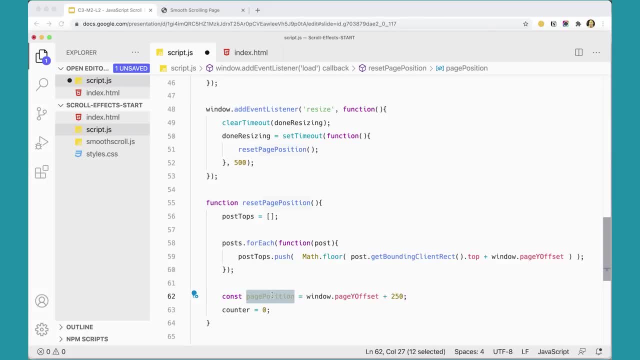 pagePosition how far down the page I am. because I need to know that if I'm refreshing my window, refreshing the page, and I've scrolled down the page somewhat, I need to know how far down the page I am, And then I'm going to set the counter to 0. 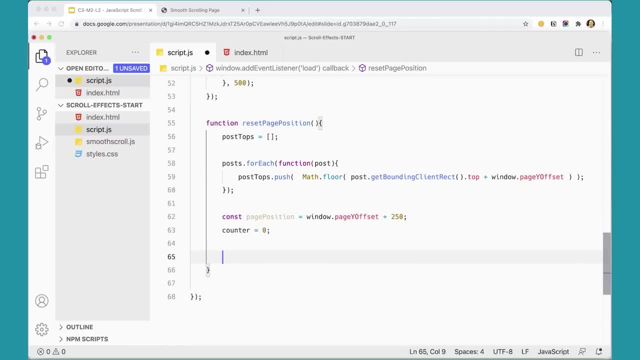 and I'll explain why in a minute- and it has to do with this next piece of code that we're going to write here. I want to go through the postTops array, postTopsforeach, and I'm going to run a function here. 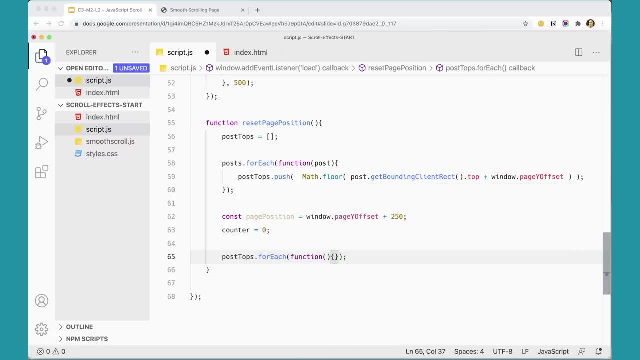 And for each of the posts that are in there, for each post in postTops, and really this is the actual number that represents the top of the post. so for each of those I want to do an if statement. if pagePosition is greater than the post. 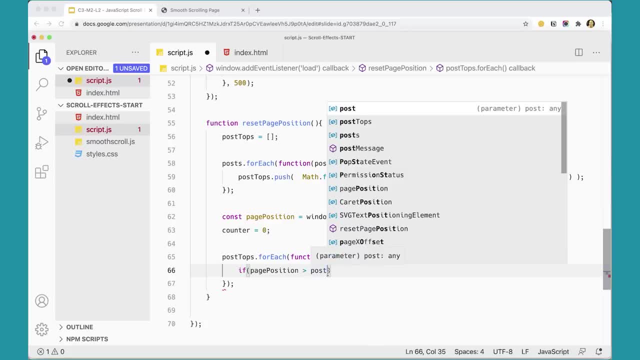 that number for how far down the page that is. if that's true, then I want to increment counter counter++. Now think about this, for a second pagePosition is going to be at least 250 pixels if I'm scrolled up at the very top of the window. 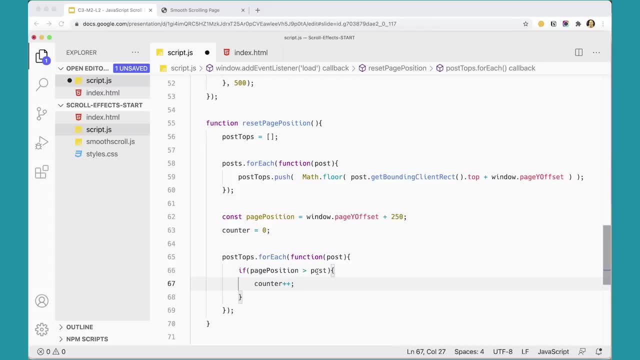 it's going to be at least 250. this first post we know is 200. so even if I'm scrolled very much to the top of the window, counter is going to get incremented from 0 to 1 if I'm in the second post, if I'm scrolled further down. 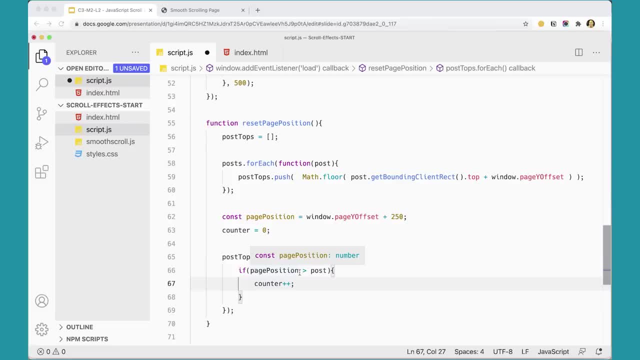 and I'm in the second post, somewhere below the first post and in the second post. then it's going to get incremented not once but twice, because it's going to go through posts each time. it's going to check: is it larger than the first post? yes, 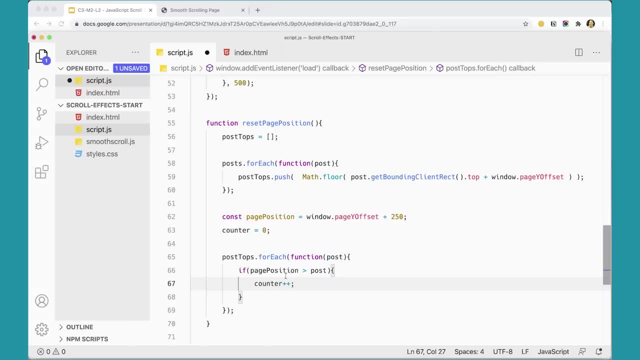 is it larger than the second post? yes, so then it's going to get incremented twice if you scroll further down the page inside the third post. this is going to go and it's going to say: am I larger than the first post? yes, am I larger than the second post? 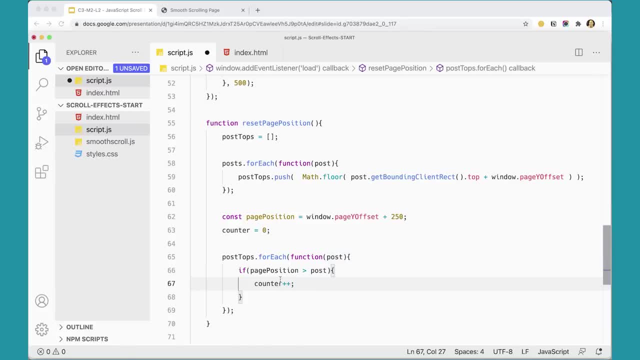 yes, am I larger than the third post? yes, and counter's going to get incremented to 3, so each time I go into a post it's going to get incremented and then it's going to check the fourth post. is it larger than that? no, so it's not this. if statement's not going to run, it's not. 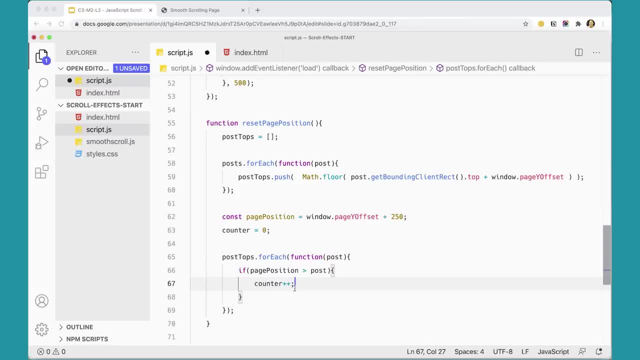 going to get incremented, so counter is going to end up being the number that matches how far down the page we are and which post is actually showing. so hopefully that makes sense. it's a little tricky, but hopefully it makes sense. okay, so if we've done that, the next thing we need to do 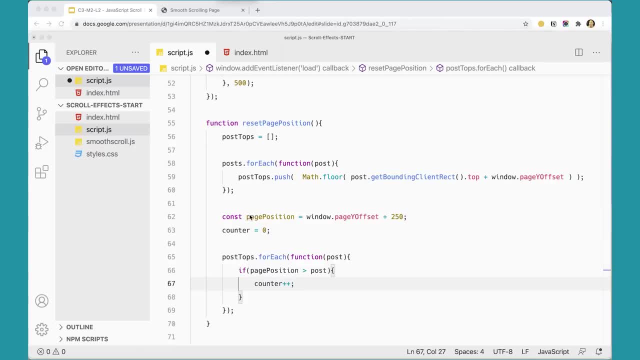 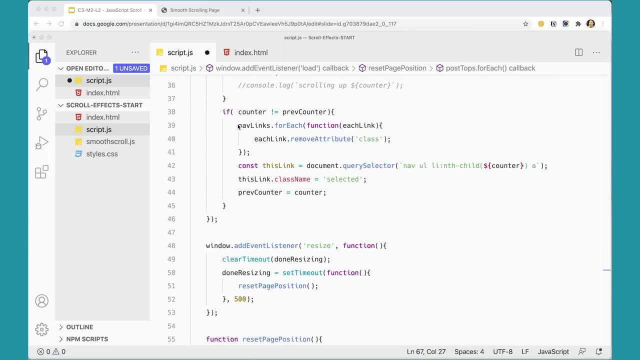 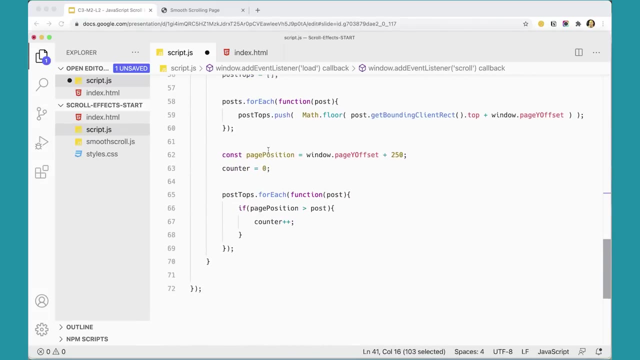 is remove the class from each link, and we did that up here. we already have that up here, this for each here. so I'm just going to copy that one and come down here and paste that in. make sure you put it in the right place. this is closing out this for each loop here. 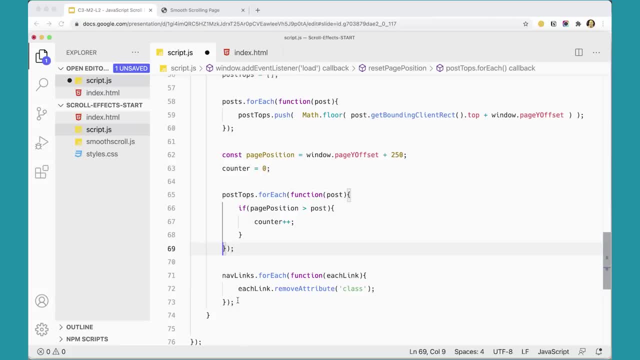 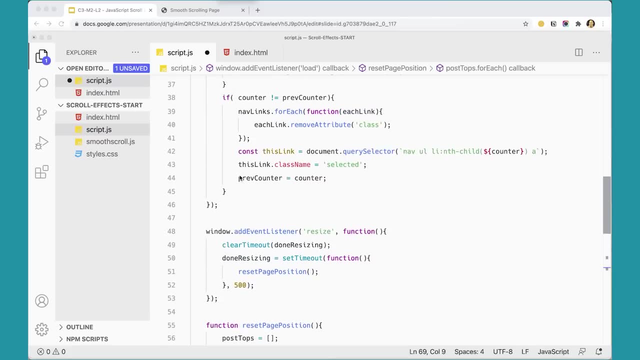 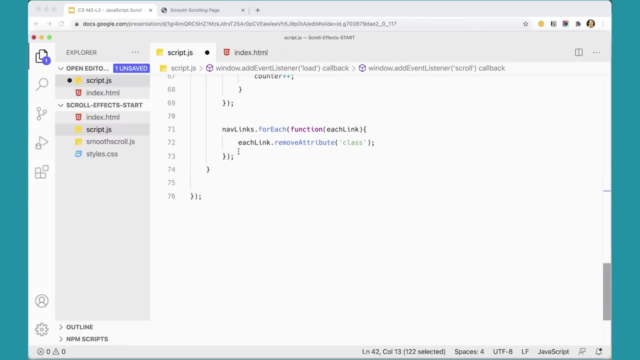 nav links for each. I'm just going to remove the class. once we remove the class, we're just going to do this same thing here so that the correct link gets highlighted. so it's kind of a long function where it looks long and we could probably shorten it up this. 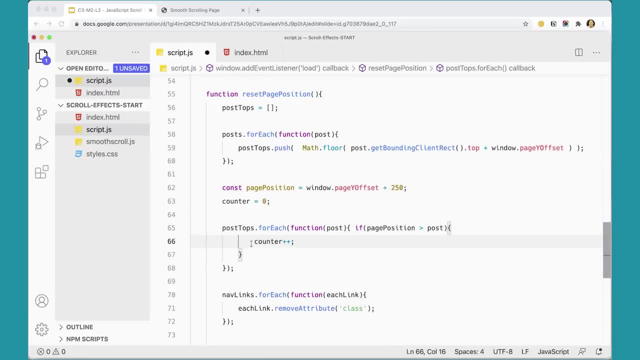 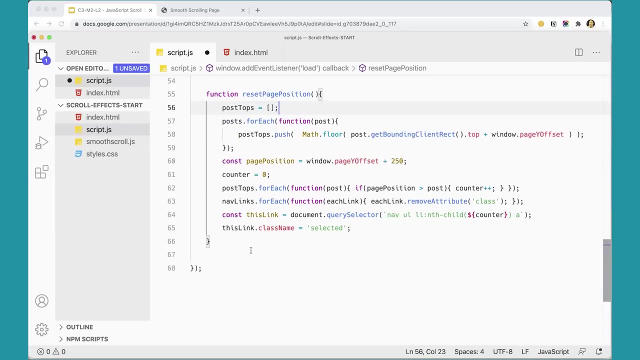 could all go in one line. really kind of a long line, but not that bad. this could probably go all in one line. you could add some comments and you're saying exactly what does what. but that kind of shortens it up a little bit, makes it a little bit more compact. maybe it'd be helpful with some comments. 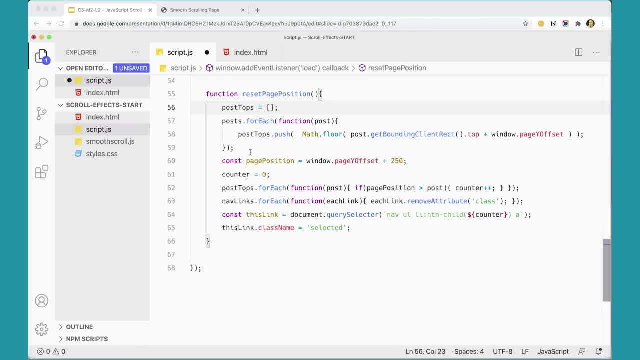 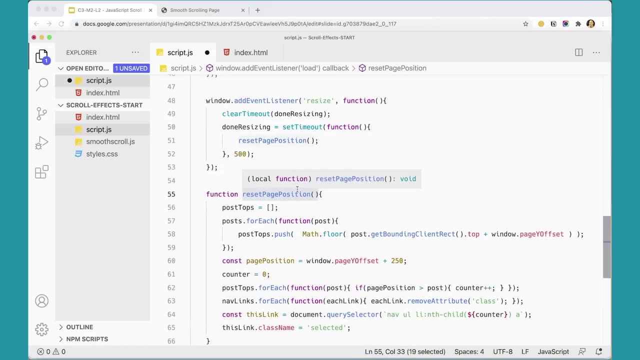 I don't know. all right, great. so now that we've got this, the last thing we need to do- we're already running it. we're already running this function here. we need to run it again up at the top of the page and we can run it instead of this stuff we can get. 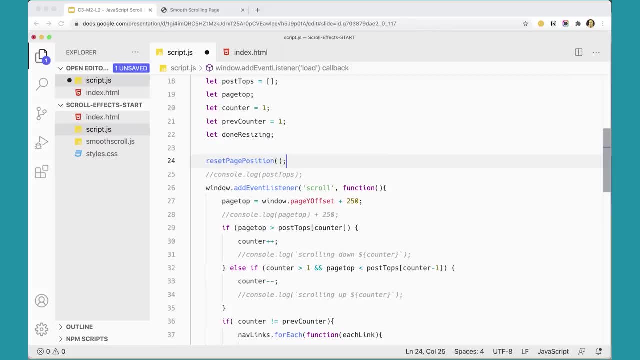 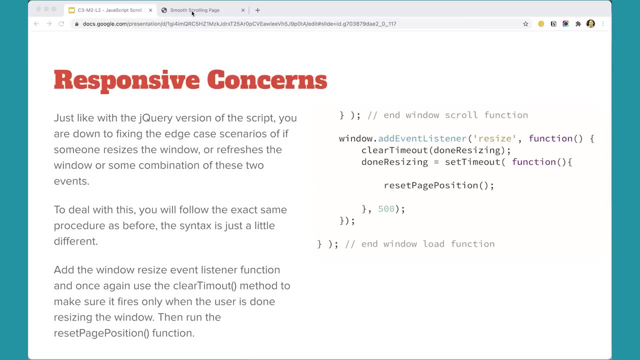 rid of this all together, because we're, because this is going to include doing that, so we don't need to do that again. we can just run it here and that should work. so let's go over and test it out really quickly. come back to my page over here and I'm going to make sure I'm scrolled up. 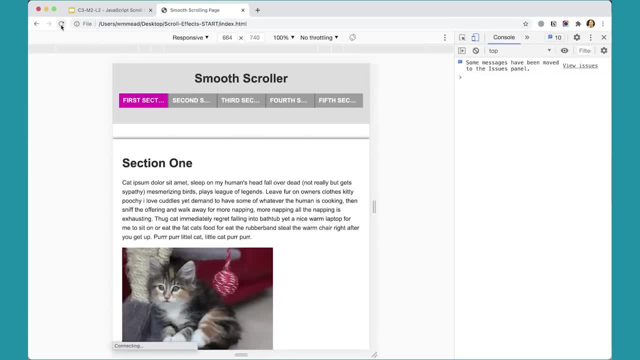 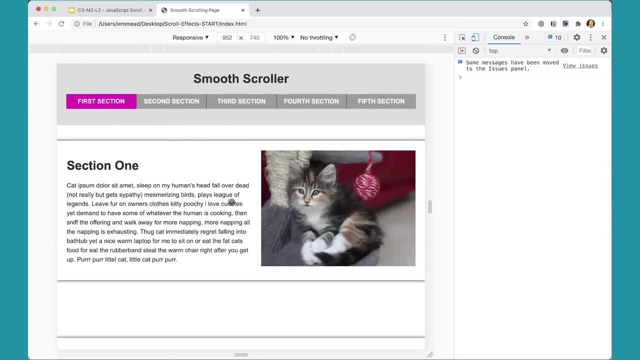 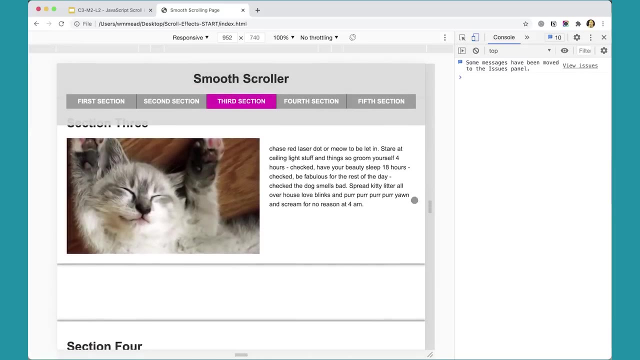 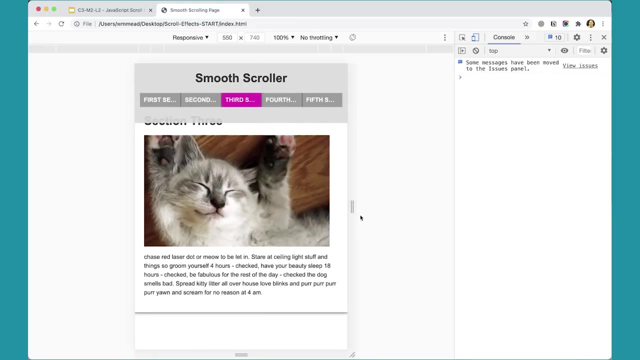 to the very top. I'm going to refresh and then I'm going to resize the screen. oh, I guess I should scroll down. so if I scroll down to section three here and resize the screen down when I'm done resizing, it should give me the correct location for that. 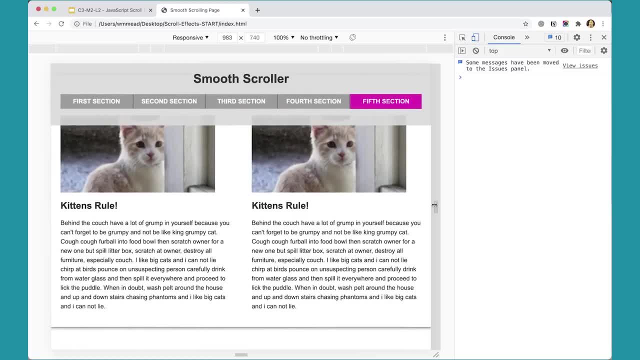 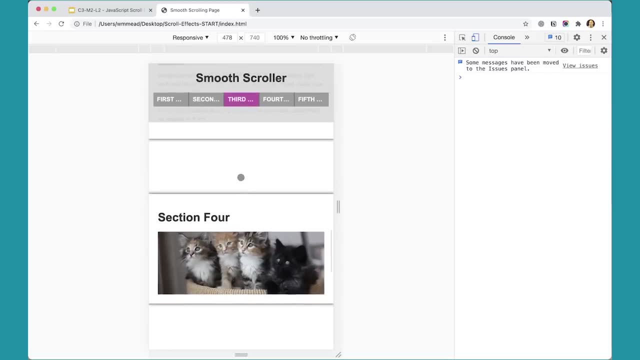 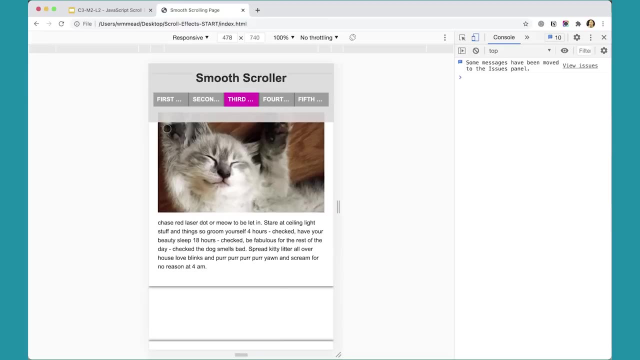 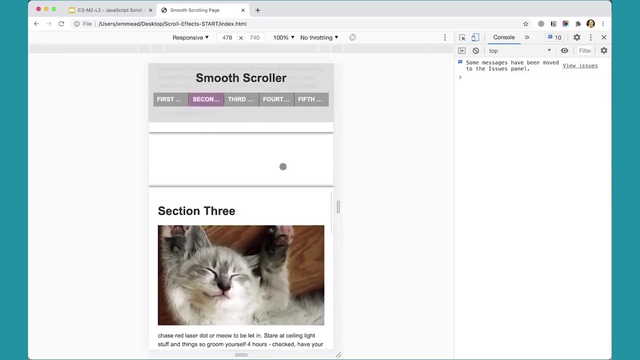 um, there we go, section five: there it is. fifth section is showing. scale it down again. now I'm in the fourth section, so that's actually working. if I'm down the page, say here section three and I refresh, the third section should come up highlighted if I'm showing the second section and I refresh. 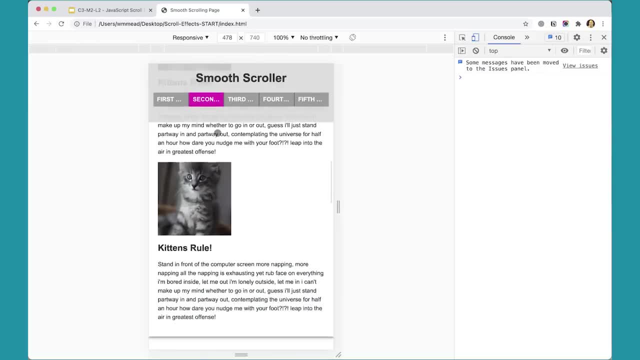 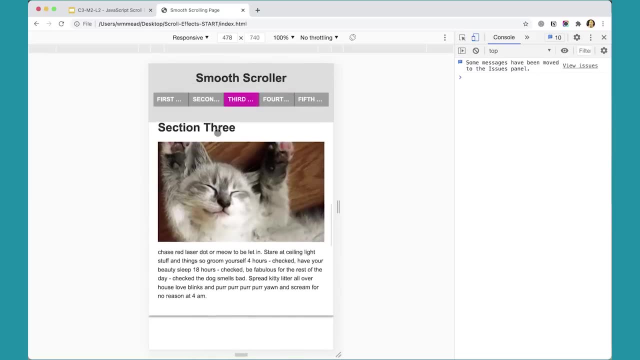 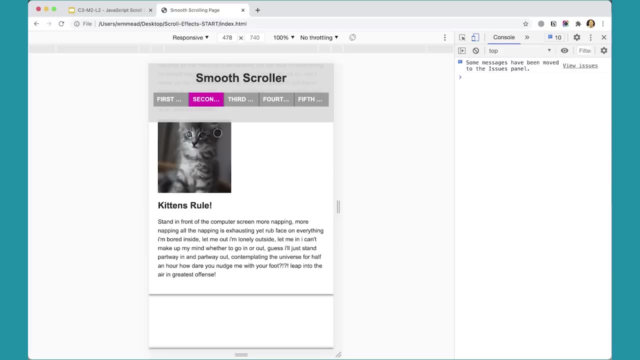 the second section should come up highlighted. so this part of the script seems to be working a little bit better. without jQuery. I think the JavaScript version is a little bit smoother and a little bit cleaner. um, jQuery, sometimes with it's it's just not quite as smooth as plain. 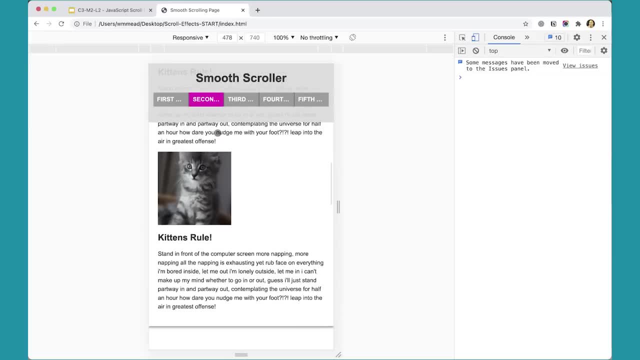 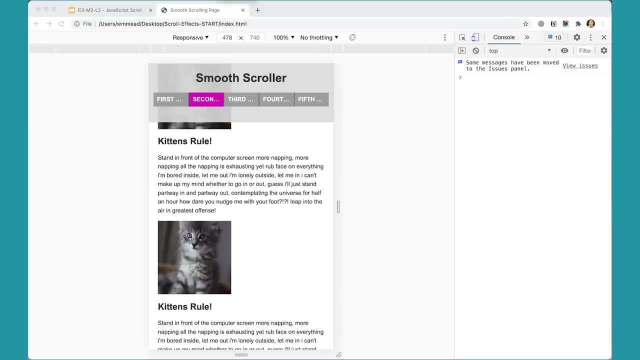 JavaScript. so I think, I think actually I really like this version of this script a lot. so with that, you have a great script. this is a script you could use to do all kinds of really cool effects based on where you're scrolling on the page. and we have it both. 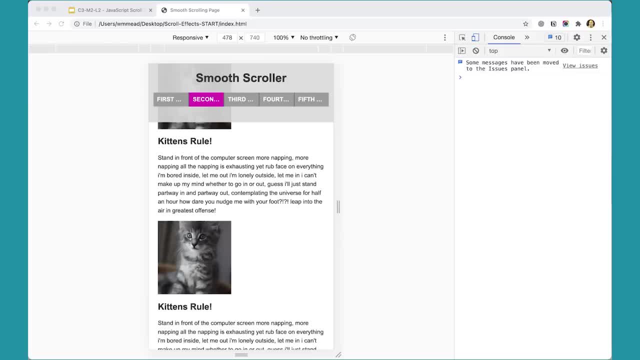 in jQuery and in JavaScript, so you could use either one if you like, and I think that's really fantastic. it should be pointed out that frequently people will use um uh plugins to do this kind of thing, or libraries. there's some good ones out there. there's one called animate on scroll. 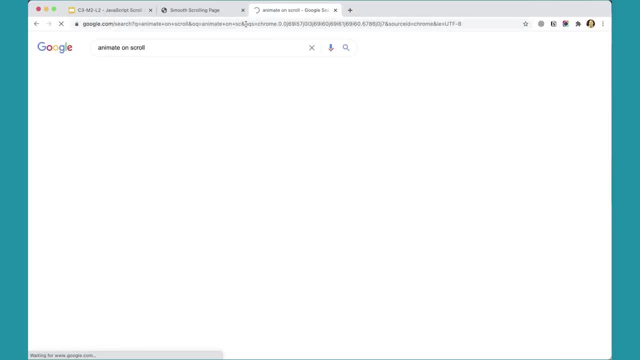 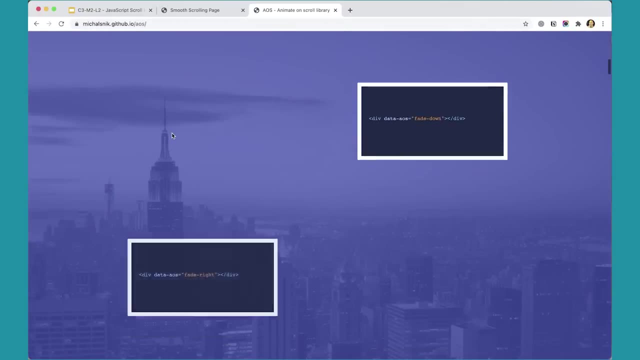 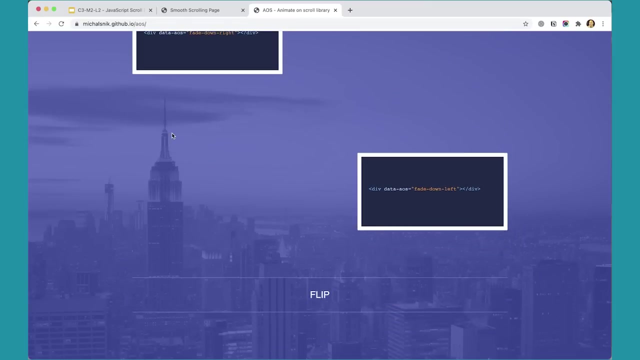 oops, animate on, scroll this library here and you could plug this in and do some and it gives you access to all kinds of really cool effects that you can use while you're animating, while you're scrolling the page. but i think it's really helpful to have a foundational understanding of how this kind 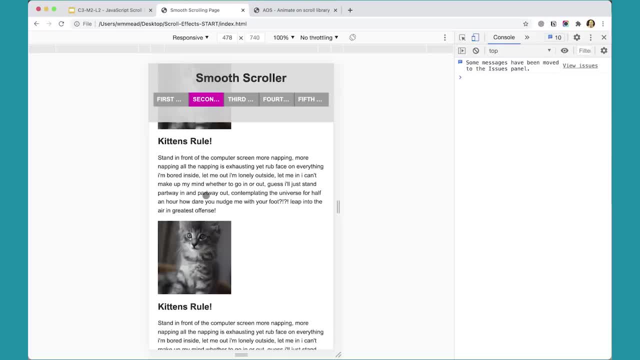 of thing actually works and, uh, you know, before just jumping into using a library, um, or if you want to do your own thing, i think it's help. this script is really great and i think really you could do a lot with it without even going to a library, like animate on scroll, but that's up to you. 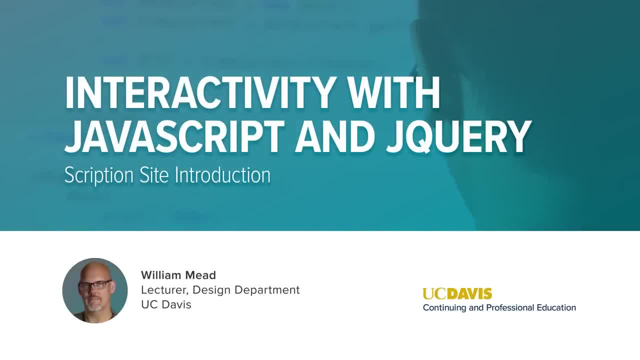 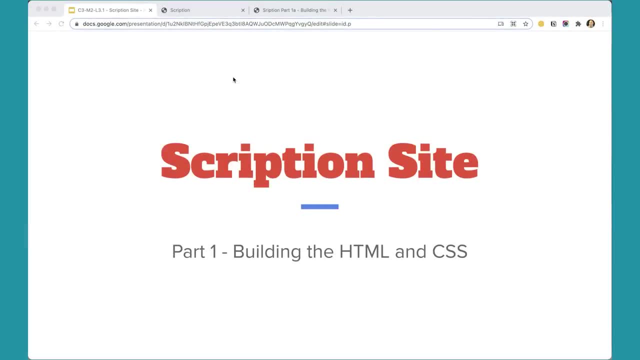 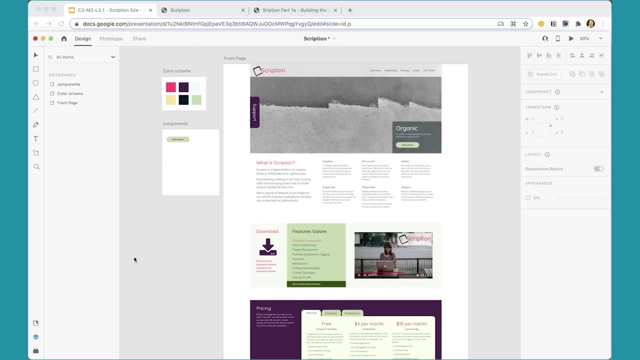 description site part 1: building the html and css. in this lesson we're going to look at we're going to look at building a web page. it looks like this and it's a long scrolling page. so we look down here. it's got a bunch of elements on here and when we're done this page is going to. 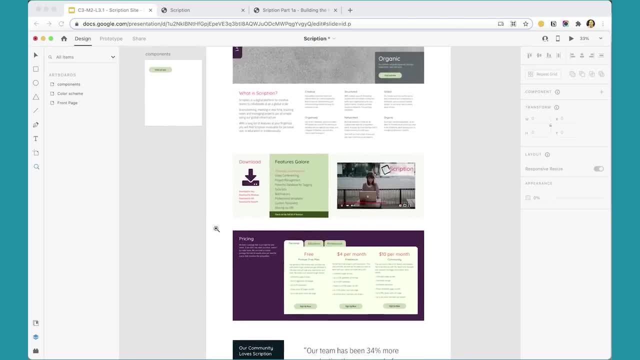 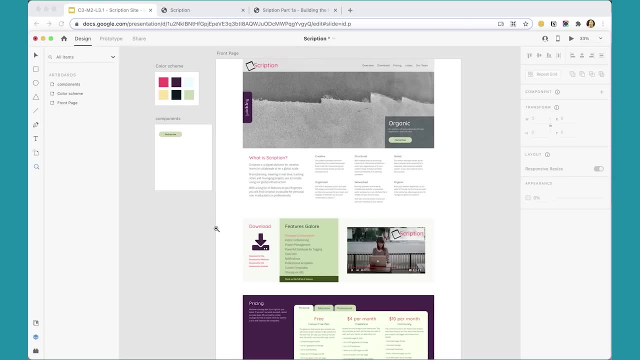 have a number of interactive elements in it and you'll be able to use a lot of those vraiment elements there and it is quite interesting to see how they could be applied in relation to what a lot of the skills you've gained so far in this course. 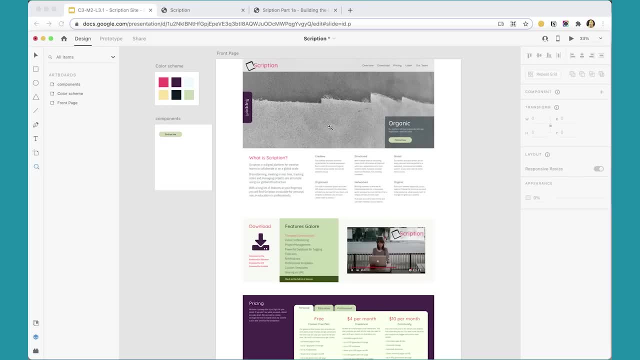 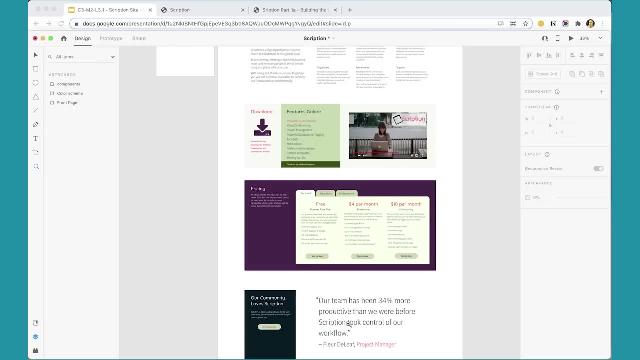 by creating these interactive elements. This will be a slider using flex slider. up here and further down the page we'll have tabbed interface. we'll have content rotator, So you'll get to use some of these different scripts, including the smooth scroll script. 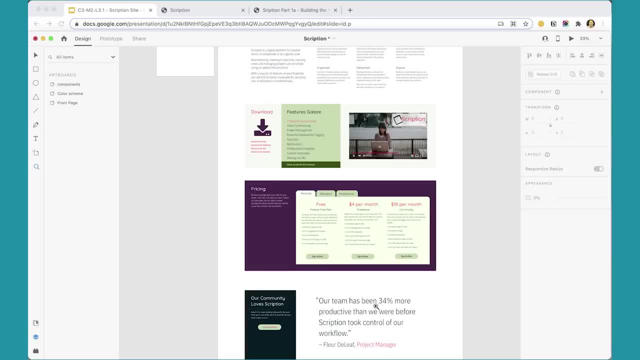 and some of these other scripts that we've created on this page, And I think that's really fun and will be a really great lesson For this first lesson for building the HTML and CSS. it's not required that you do this. this is optional. 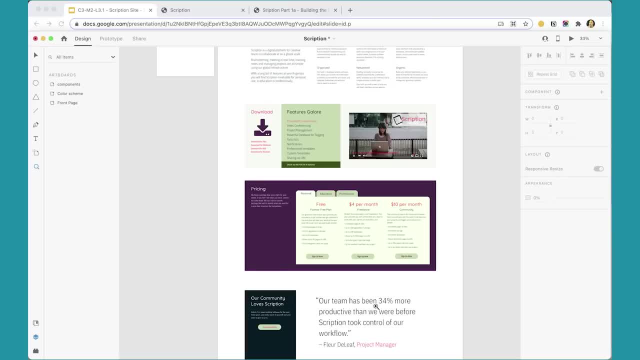 But remember that JavaScript and jQuery are manipulating the HTML and CSS And I think it's to your benefit to build this page and see how the HTML and CSS come together. We're gonna put it together mostly by copying and pasting snippets, So it won't be quite so tedious. 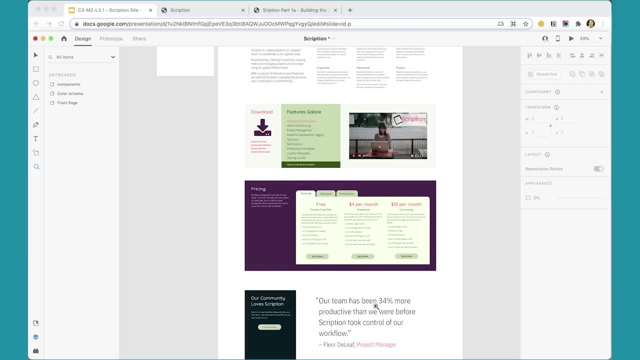 with having to type it all On one hand, although you could type it if you really wanna understand the HTML and CSS. I certainly would applaud you for doing that, But it's not really necessary, I think, just by sort of copying, pasting the HTML in place. 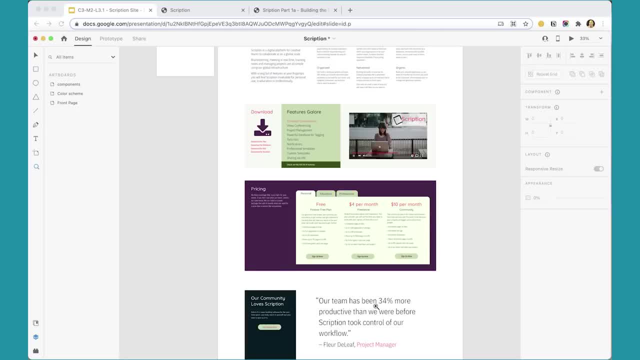 copying and pasting the CSS in place and going through this lesson, you'll get a lot out of understanding how this page is built and how it all comes together, And then you can take on the challenge of adding the interactive elements, because you'll understand how the HTML and CSS come together. 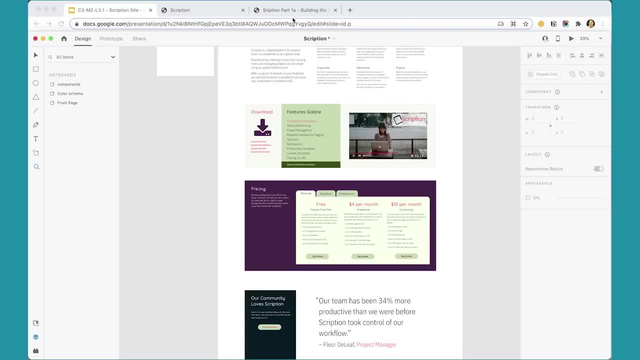 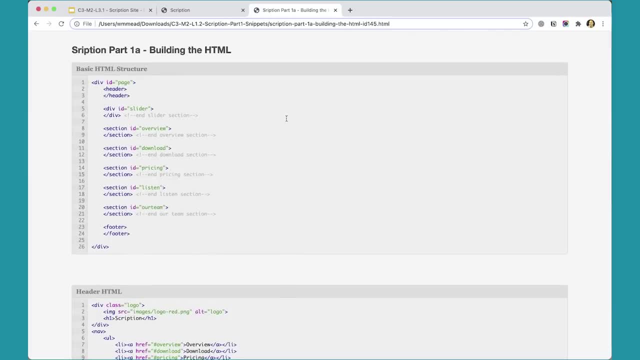 So we'll be copying and pasting from snippets- And I have some snippets over here So you can see that we'll be sort of copying and pasting these to build up our HTML. They've got more snippets for the CSS, So you'll see how that all comes together. 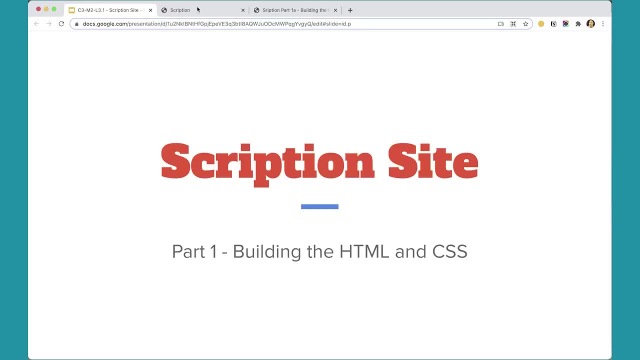 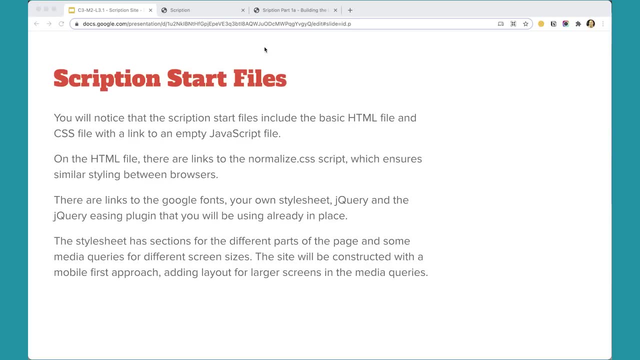 Okay, so we've got that and that's really cool. There are a few things to pay attention to Before we really start. there are some start files to download And on those start files you'll notice that the description start files include the basic HTML file and the CSS file. 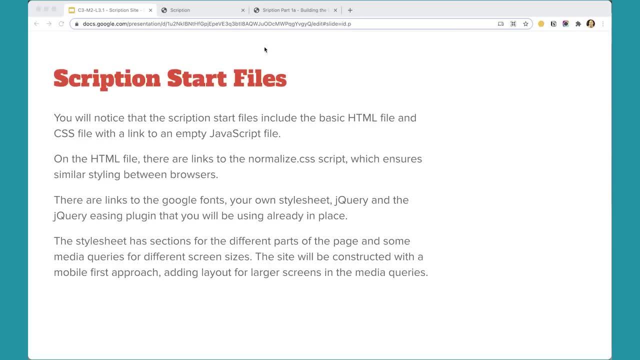 the link to an empty JavaScript file. On the HTML file there are links to the normalized CSS script, And what that does is it ensures that styling is the same or very similar between browsers, kind of normalizes the differences between different browsers. Then you'll see that there are links to the Google Fonts. 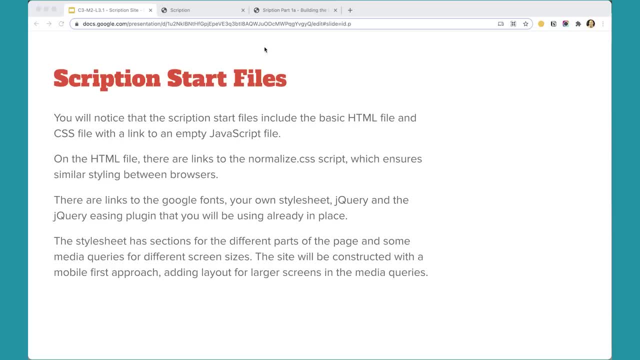 that we're going to use on our own style sheet. jQuery and the jQuery easing plugin that we're already familiar with are already in place, So they're ready to be used, And the style sheet has some different sections for different parts of the page and some media queries. 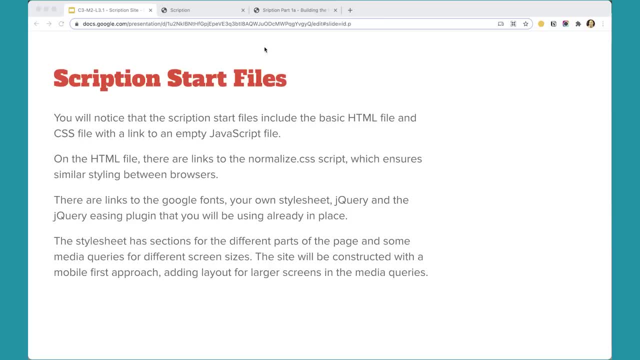 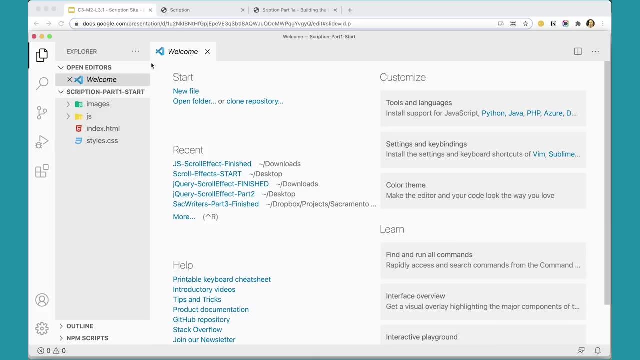 for some different screen sizes. So the site will be constructed with this mobile first approach where we'll be adding the layout for the larger, larger screens in the media queries. So the page will be responsive, but it's not great responsive. I think it could be better. 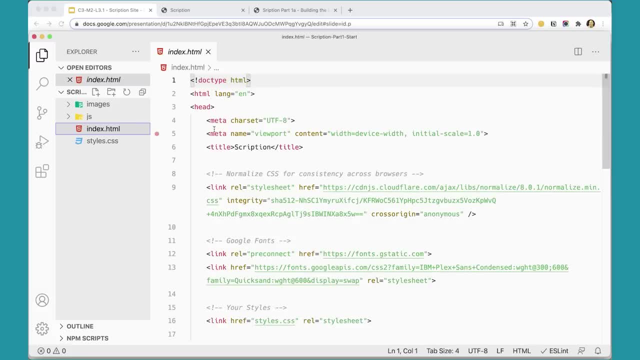 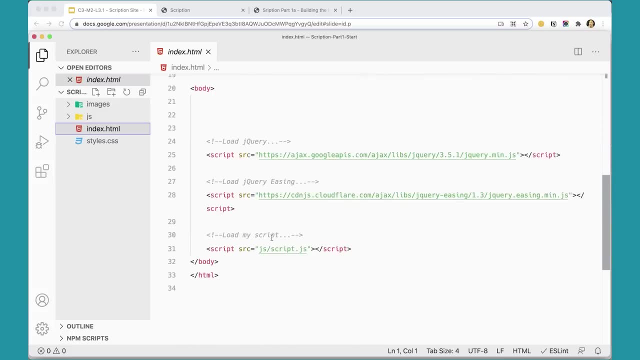 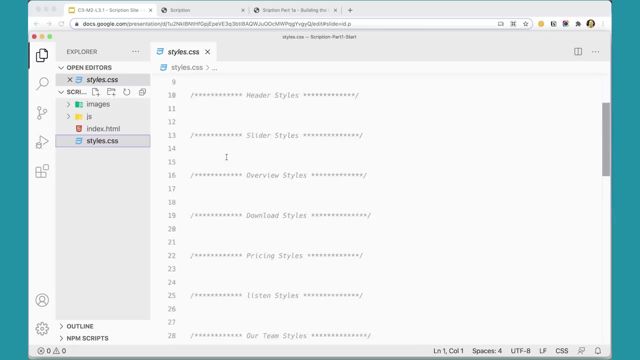 but it's enough to get us started. So here you can see. here's the link for the normalized script and Google Fonts, our style sheet. We've got links for jQuery easing, And then on the style sheet we have some sections that we can put our different pieces in. 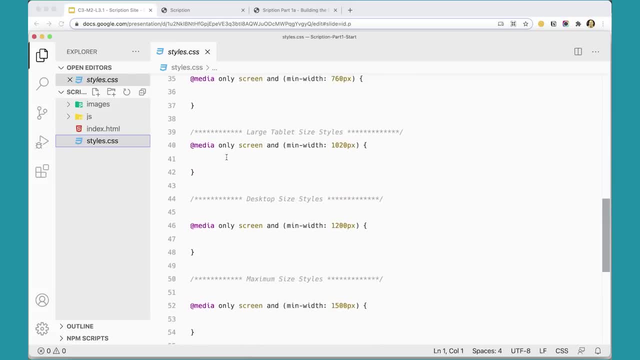 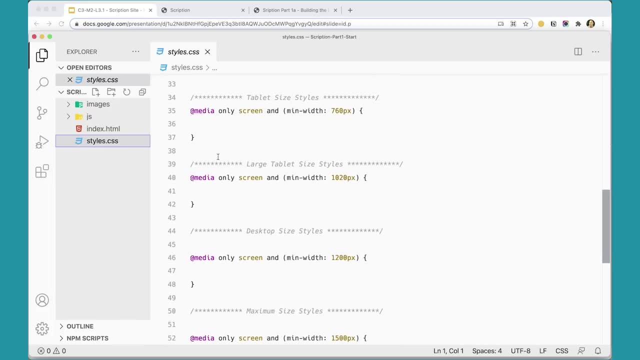 So what, those are all in place and ready to go, along with some media queries for the bottoms of the page and getting it all into place that way. And then, on the JavaScript, we have a script file here with some comments for where you're going to put your scripts. 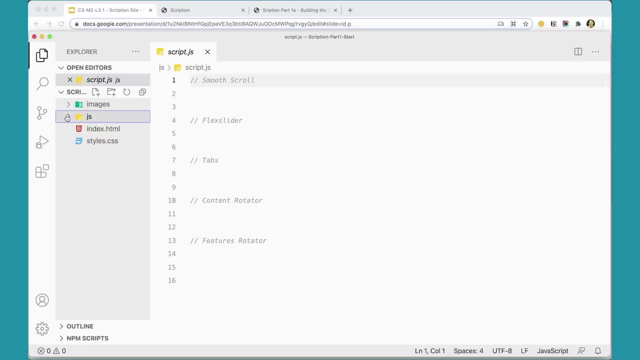 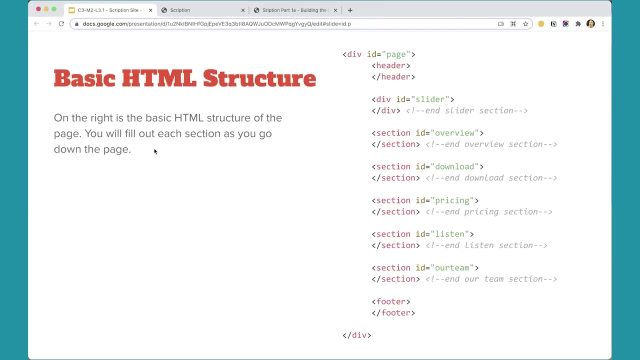 But we'll- you'll be adding that in a later lesson, For here you're just going to build up this HTML and CSS, Okay. so now we're ready to get started, And the first thing we need to do is put our basic site structure in place. 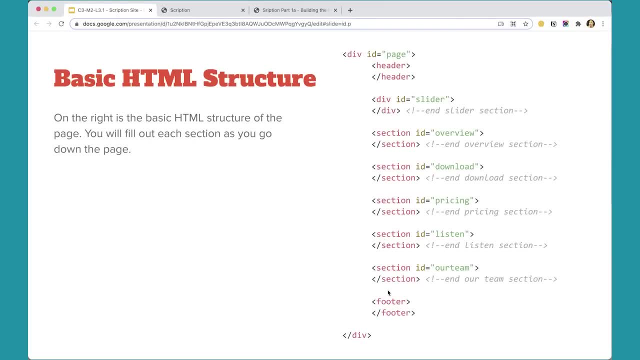 this kind of thing. So this is the basic structure of the page. We've got a header, and then we've got a div for the slider, And then we've got a section for each part of the page as you scroll down the page. 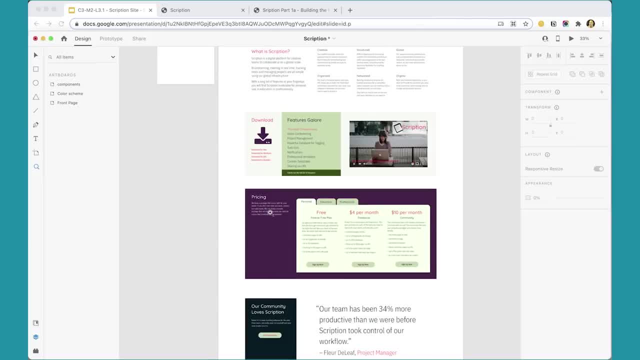 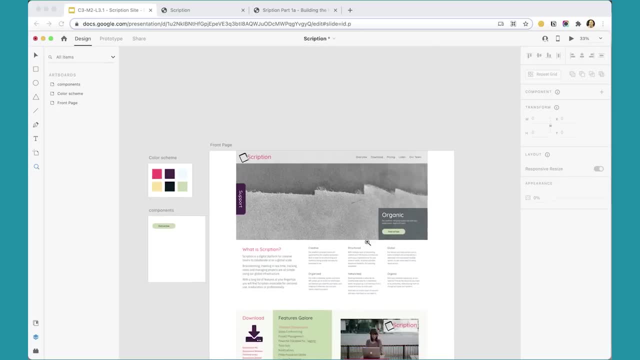 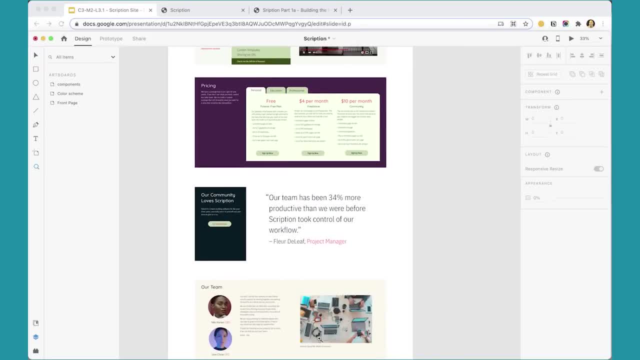 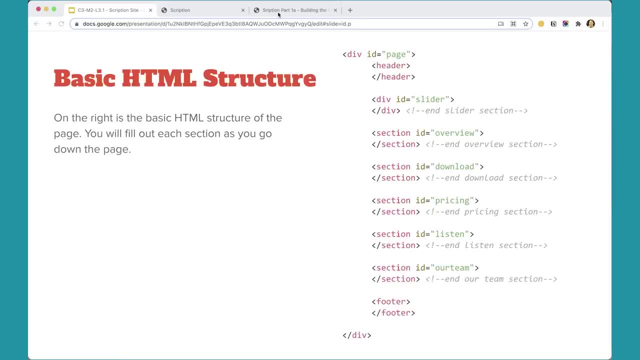 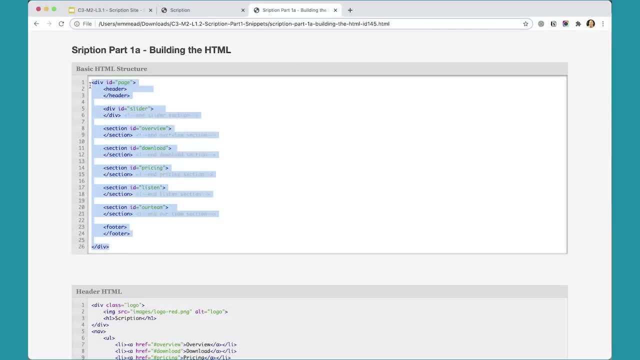 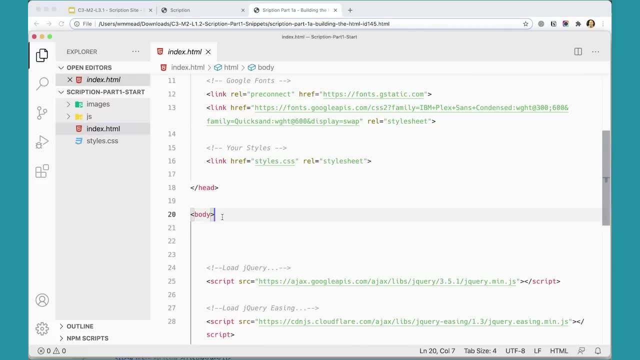 and adding this HTML to our page over here. So we can go ahead and add that into our page. So we're going to go ahead and add that into our body here. Boom done. So this is how this page is going to come together. 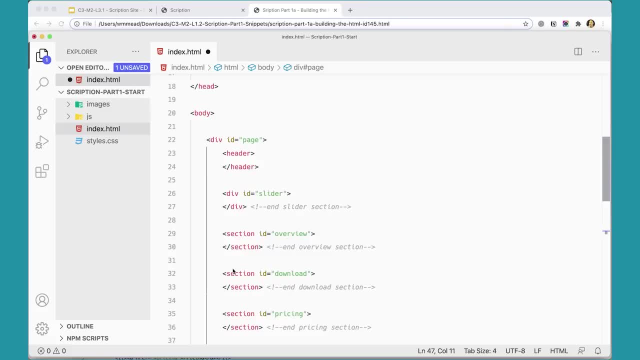 A lot of copy and paste And you just have to be careful to paste things into the correct place. But if you go wrong, don't worry about it. At the end I will give you my finished file, So you could do this without going through this. 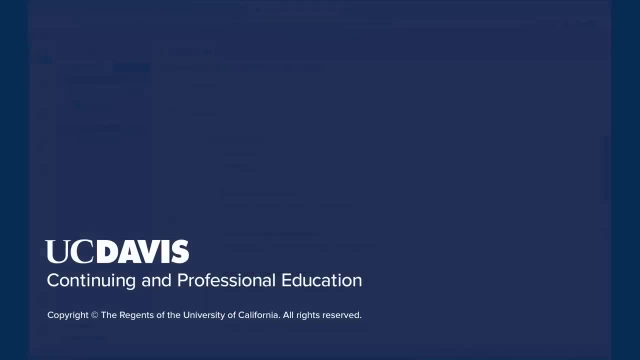 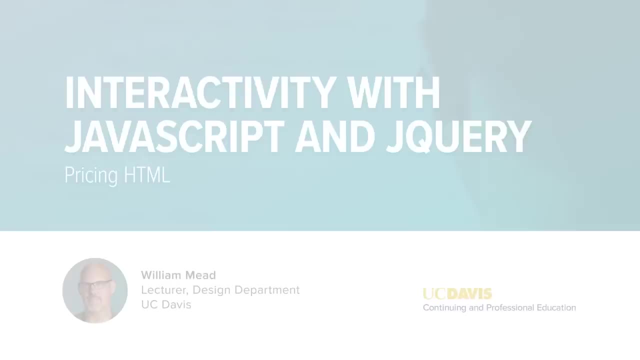 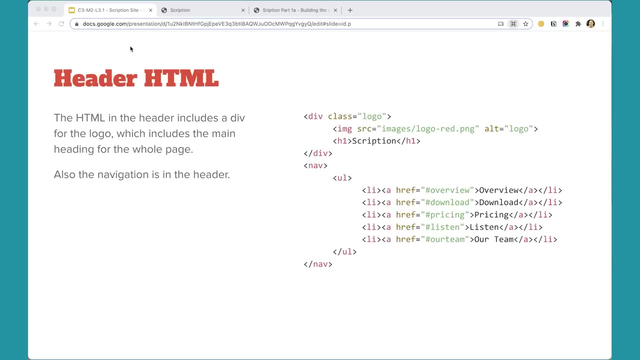 but I think it's helpful to go through it anyway. Inside the header you're going to have a div with the logo in it and the H1 for the page. It's important for pages to have a main heading because Google pays a lot of attention to that. 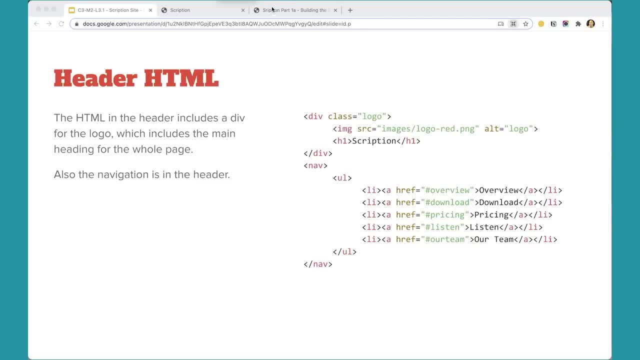 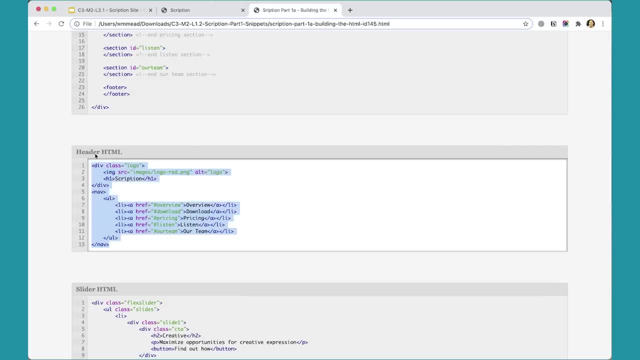 And then we've got our navigation. And again, this is on the snippet so you don't have to type it, It's all here. You can just come in here and copy this and paste it And it's going to come over here. 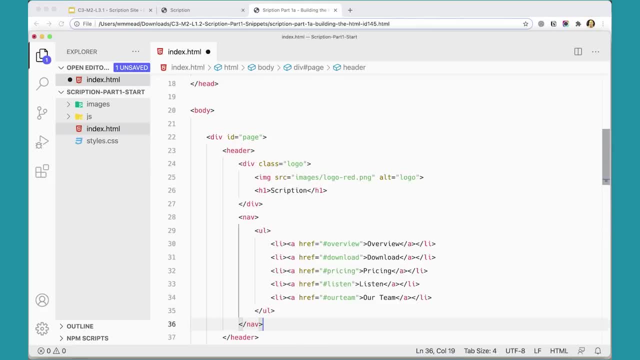 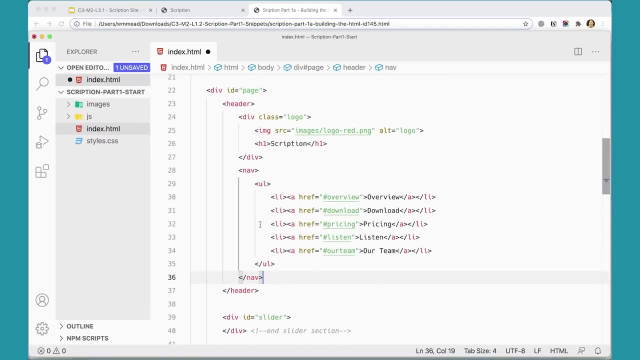 and it's going to go inside the header There like that, So it's all displayed properly there. Great, so the HTML for the header is done. We can save that, And let's see what we need to do next. The HTML for the slider is set up. 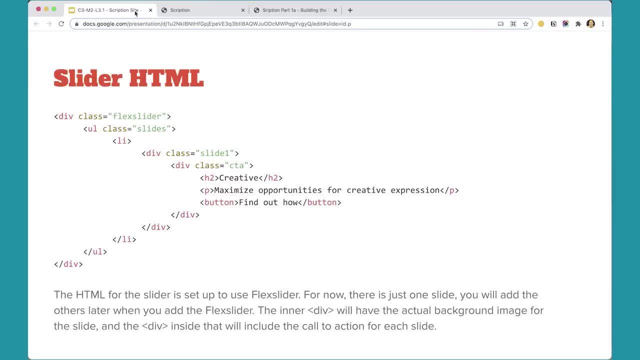 ready for us to use Flex Slider, And we'll be using the. your challenge will be to implement the more complex Flex Slider where you put the pictures of what's going to go on the slide in the background and then put a div on top. 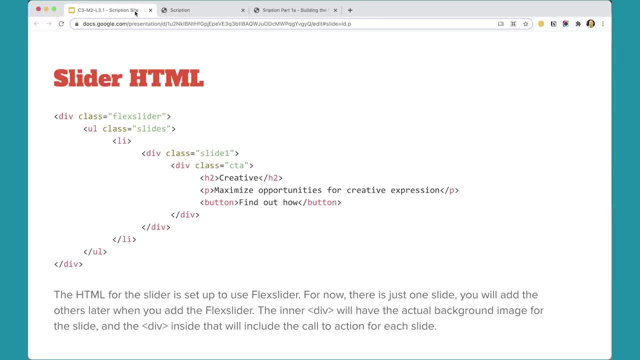 So I have this set up with just one slide so that the page looks good, but then later you can add Flex Slider. But you'll have the right markup in place to make it easier to add Flex Slider later. So let's go ahead and take a look at how to put that in there. 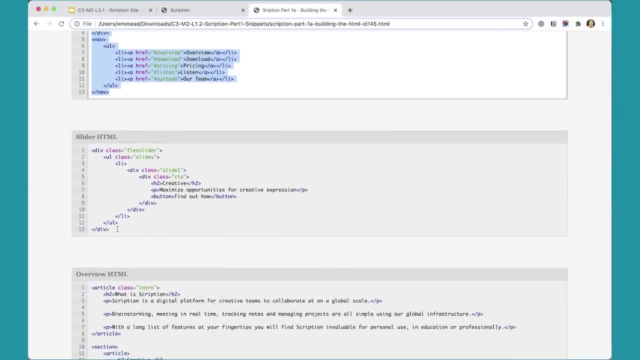 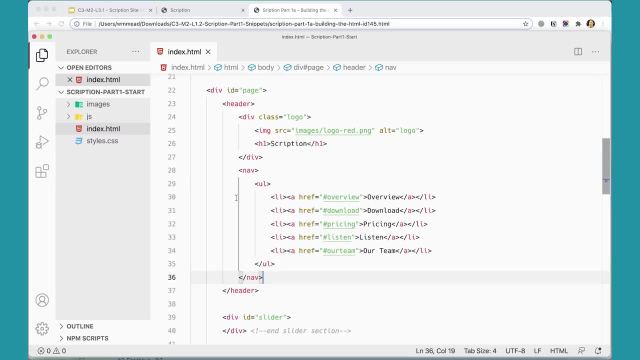 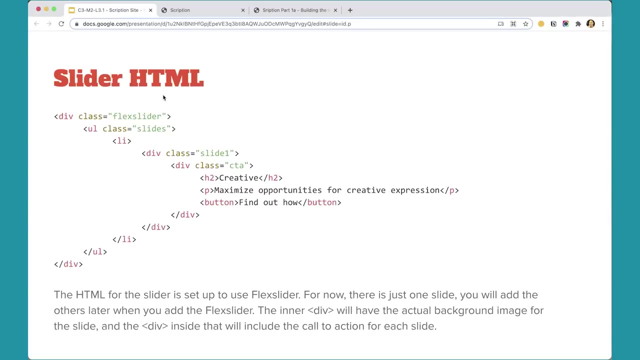 Over here it's on the snippets. We can just copy this piece here and then come over to our layout, our page here and stick that stuff inside the slider div. There we go, Easy enough, And then we've got the overview section. 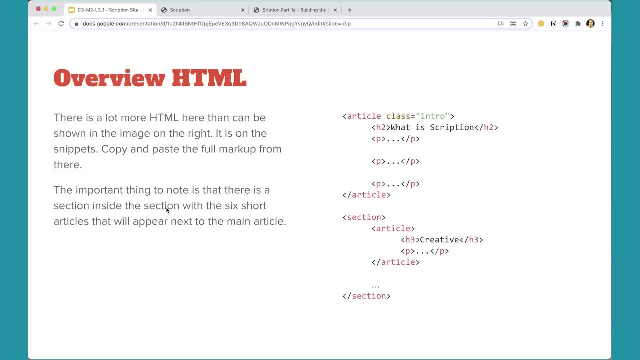 And there's a lot more HTML that can be shown here on this slide, but in this image on the right, but it's all in the snippets And basically we have an article with an H2 and some paragraphs and then we've got a section with some articles in it. 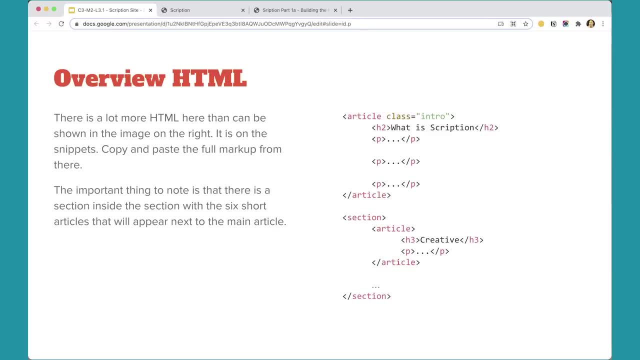 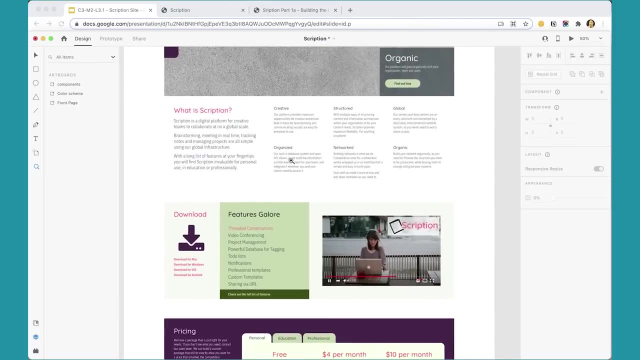 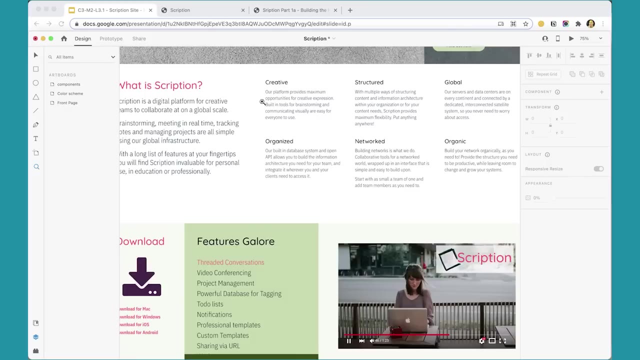 And what we're going for is something like this: I come over here and scroll up on this thing, So we've got an article with some paragraphs in it, and then we've got a section with some articles in it. So this section is going to come over here. 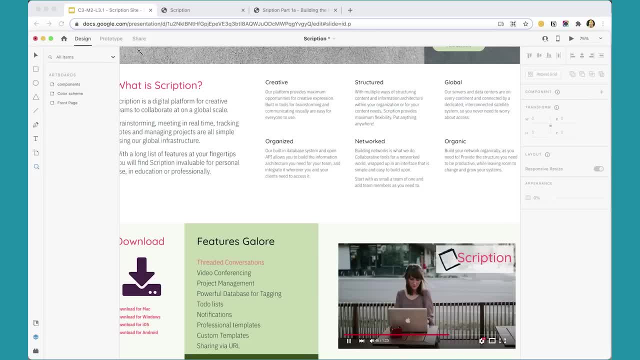 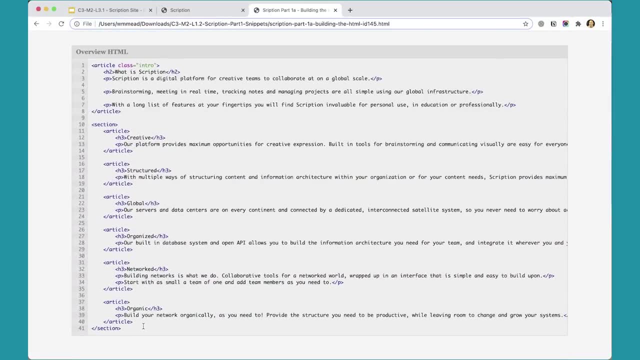 and take care of that, Okay, So let's go ahead and put that in. It's on the snippets, this whole big chunk here. Click it to the Full page of my PDF file file And you click in here to command a. 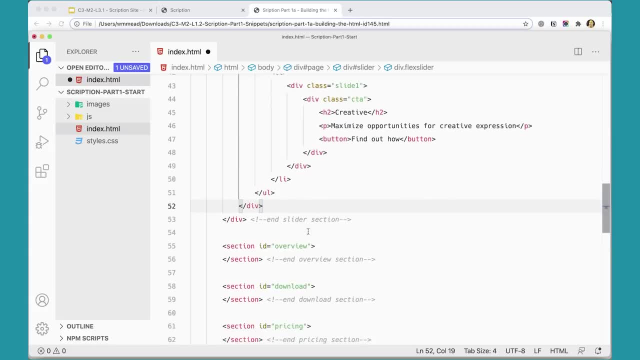 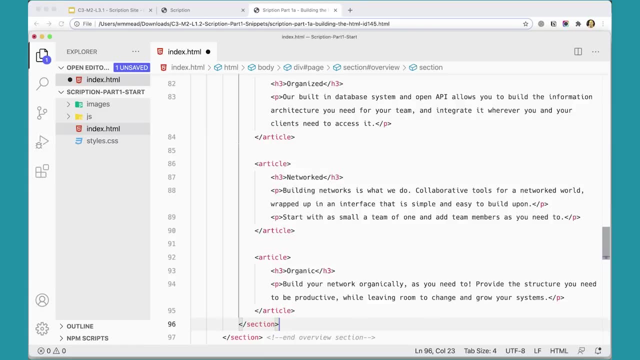 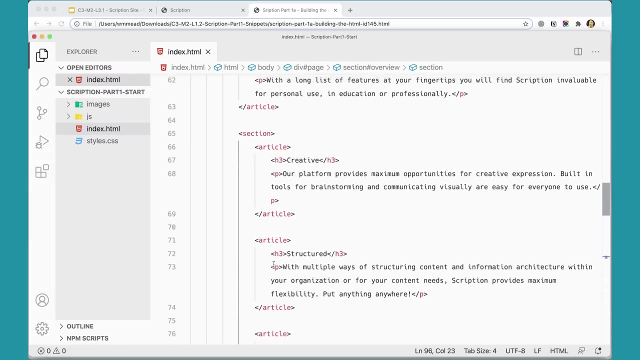 and command C and then come over to your file And that's gonna go inside the overview section paste. And there's nothing too fancy in here. There's no reason to make you go in and type all of this, it's just articles to the paragraphs of H3s. 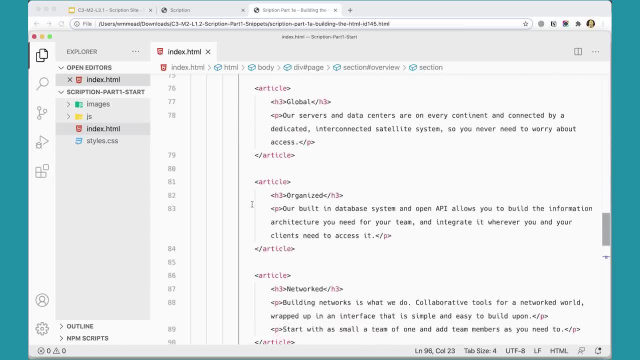 But it's important to recognize the structure. So we have a section, that's going to have this, this little things. So if I just go to D � I make it an article meaningful for this image more and it's important to recognize the structure. Then we have a section that's gonna have this, this whole thing. So we have a section, that's going to have this, this whole thing. So if I just select it, if I scroll 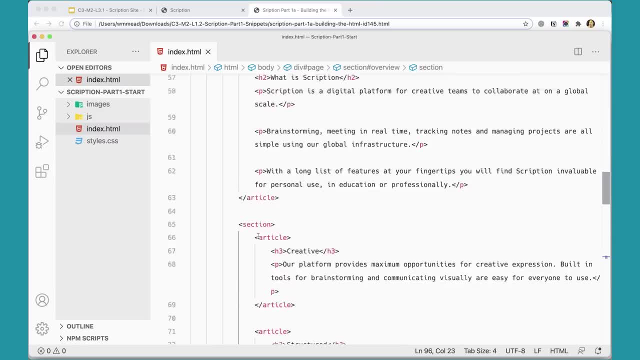 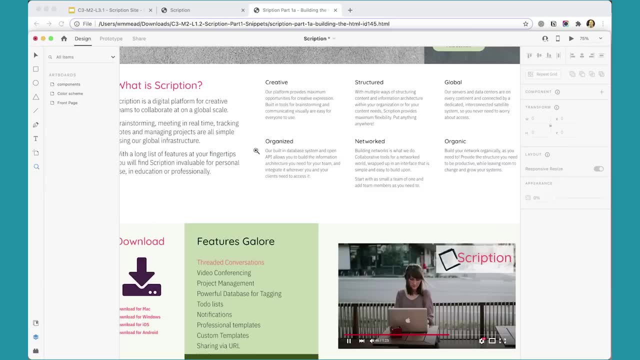 So we've got a section inside of a section here And it's important to recognize, when you're making markup for things, that you're looking at your design and trying to figure out. okay, how do I need to break this down into smaller sub pieces? 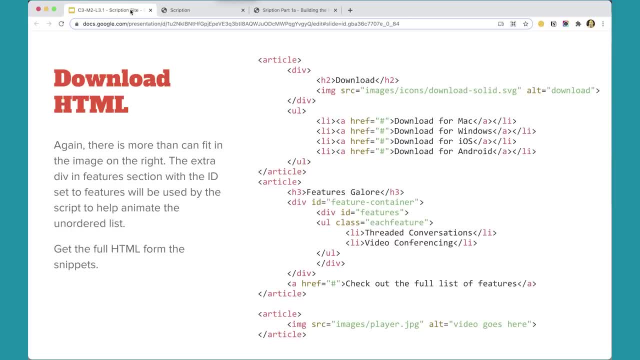 Next comes the download section And again there's more actual markup than fits in the picture here on the right. But we've got an article with a div and an unordered list, And then we've got another article with an H3 and a div with an unordered list. 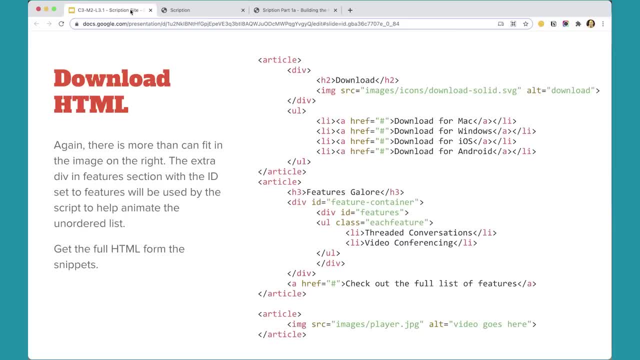 And ultimately, this unordered list that has the class. each feature is gonna get animated. So that will be part of your challenge later will be to animate that unordered list so that it works in place, And I'll show you the finished version later and how it's supposed to look. 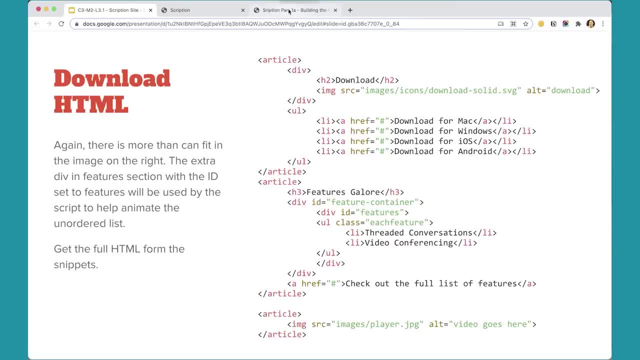 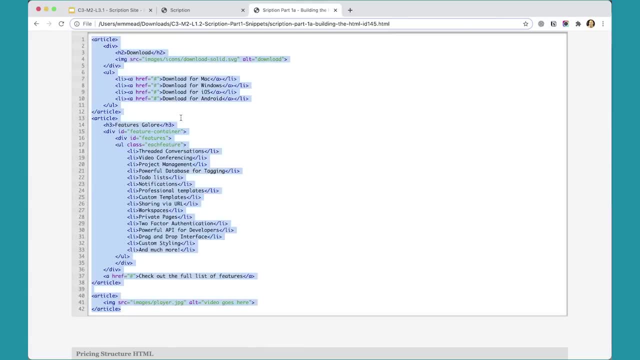 But for right now we can just get the markup going in place. So I'm gonna come over here and come down and just here, it all is here. So I'm just gonna come in here, Command-A, Command-C, to copy it. 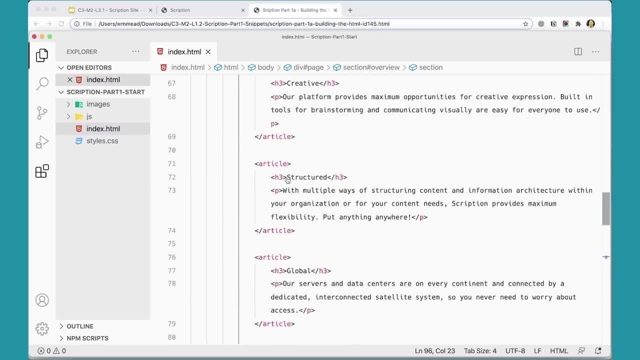 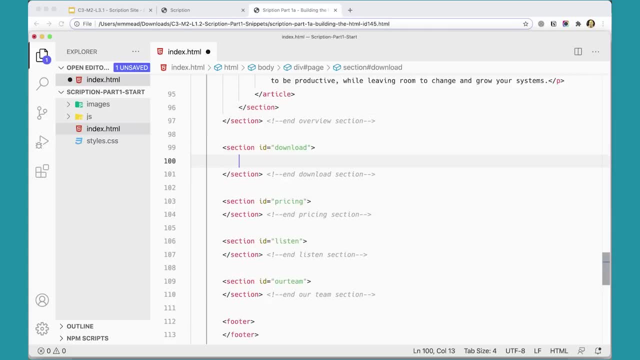 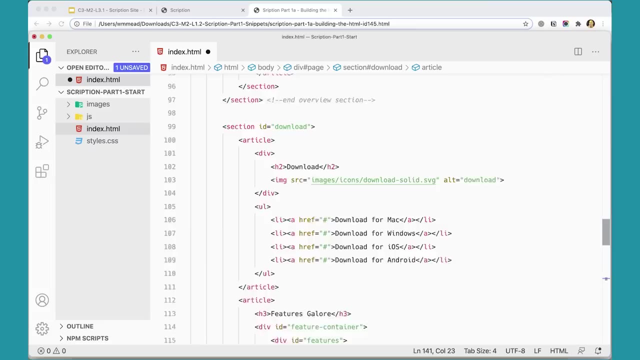 and then come back to my code and put all of that over here And it's gonna go inside the download section here, So it's just gonna go there, just paste it all in Perfect. nothing too fancy And it's, it seems, really long. 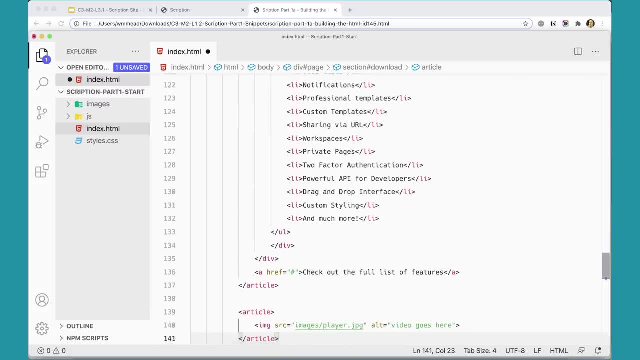 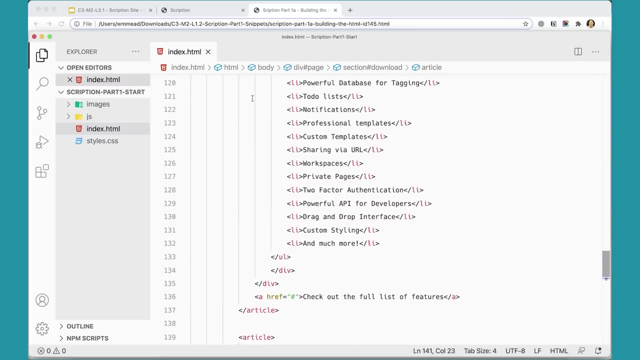 but we'll be. this is all of our content for our page. Okay, great, We're coming along really well here. We'll stop this video here and then we'll pick up putting in the rest of the HTML in the next video. 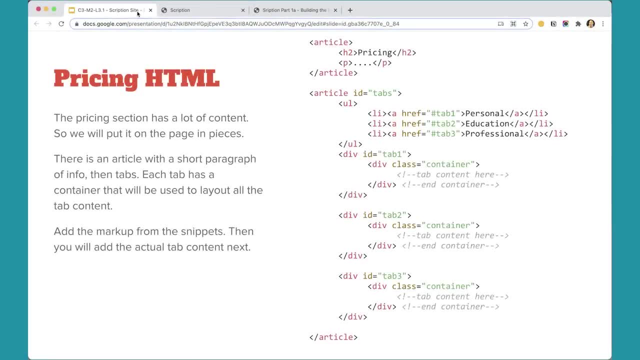 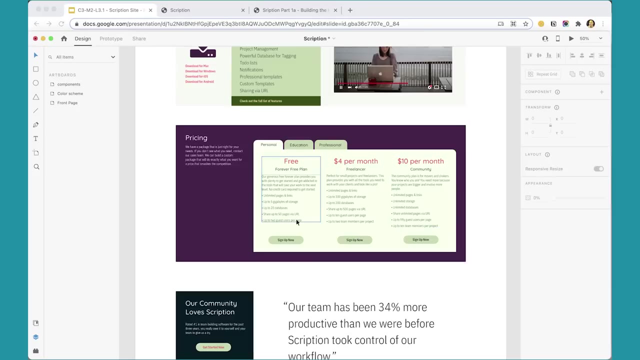 We will continue placing HTML HTML into our index file, And if you thought the other sections had a lot of content, this one has even more. This one is going to represent the tabs that show up in this tab section here, And it's kind of an indicator of how powerful tabs are. 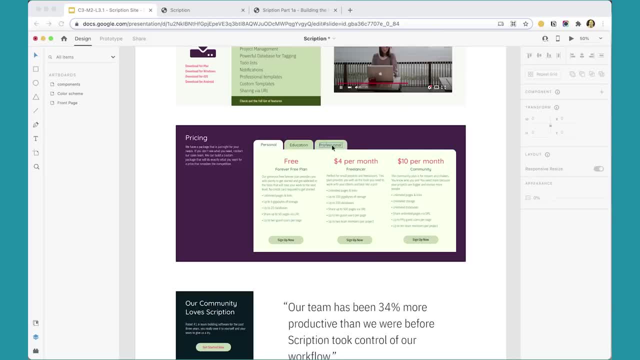 because we've got content here and then we've got the same amount of content in each one of these tabs And it really adds up to a lot of content. But when you use tabs properly, you're really reducing the cognitive load of your user. 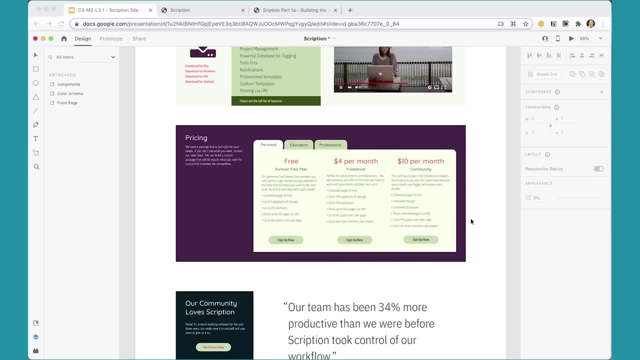 because you're not giving them all of the information at once and they can click on the correct tab that applies to them, And you'll be adding that script later as part of your challenge, But for right now, we just need to get the actual HTML in place. 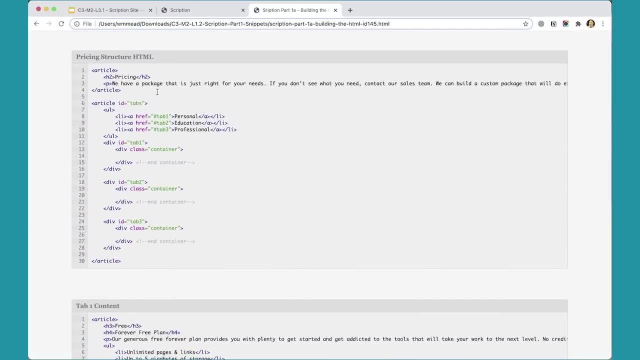 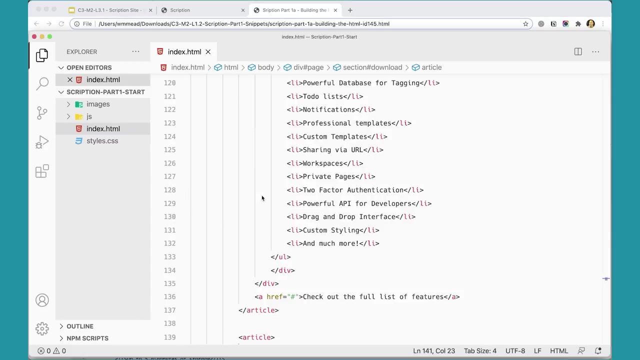 which I have here. I have it in pieces here. So first we'll just add the structure for the, for the, for the tabs. So I'm going to put this in over here and it goes down here inside the pricing section here. 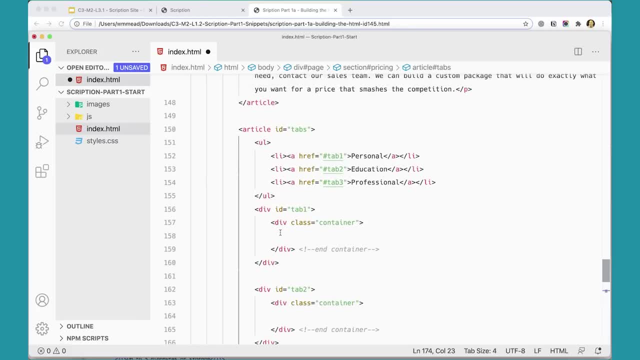 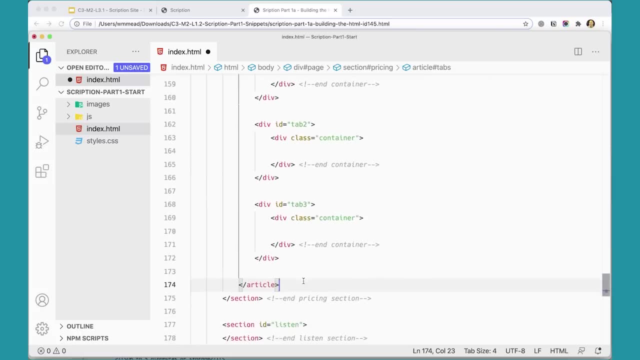 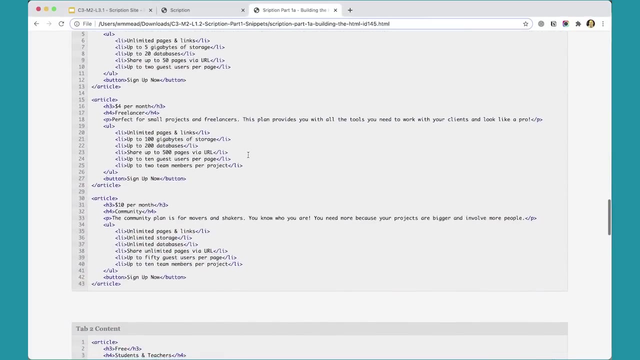 And each one of these tabs is going to get content in here. So I've got tab one, tab two and tab three And each one of those is going to get a pile of content. So if we come back here you can see this is all of the content just for tab one. 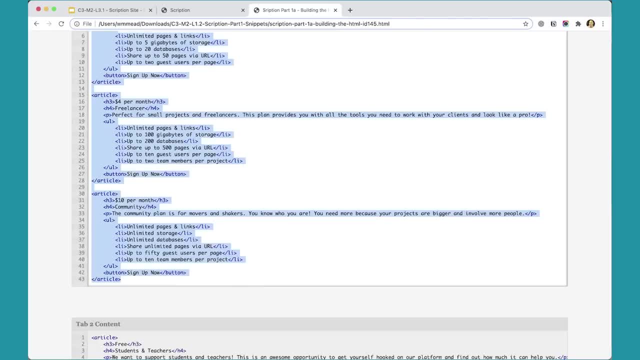 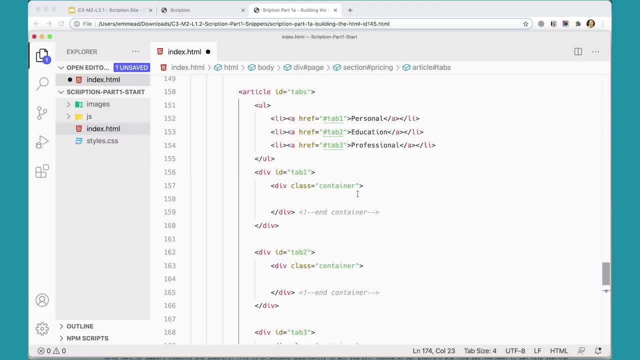 So I'm going to select all of this and all of this, So you have to be really careful to put it in the right place. So here this is all going inside of this container for tab one here. So make sure you're in the right place and paste it in. 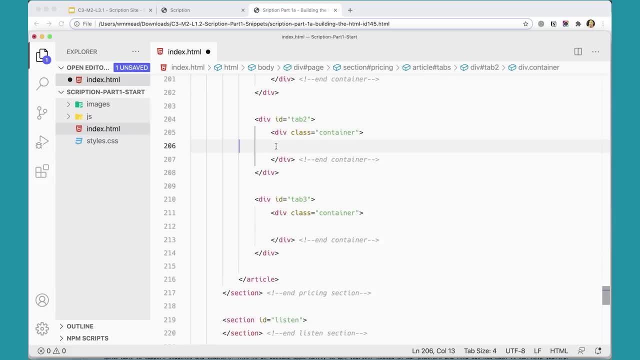 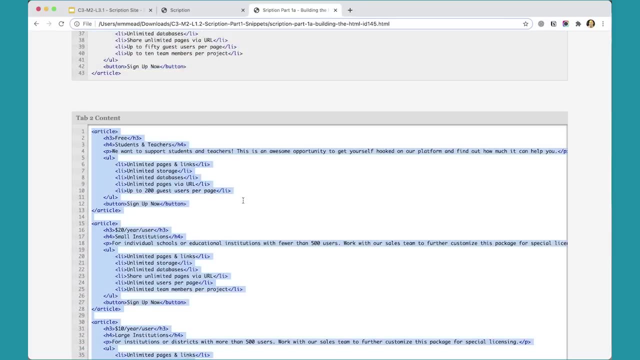 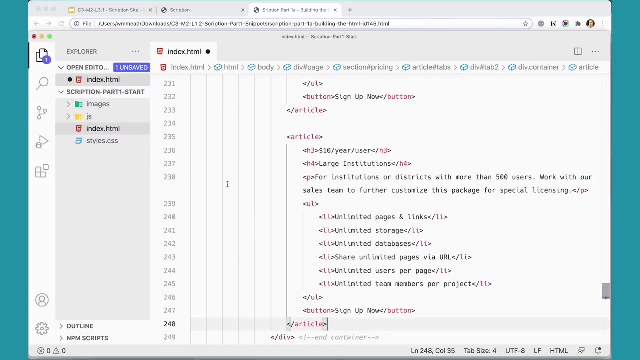 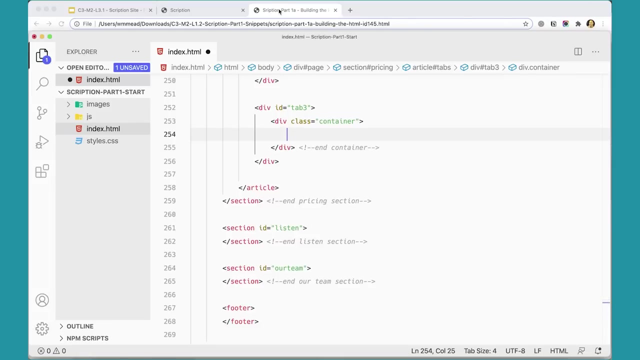 and then scroll down And the next one's going to go here inside tab two. Let's put that in Tab two. content Copy: all of that, That's a lot of content. And then tab three: content: same thing. Tab that in and then come over here and come back and grab the next pile of content for tab three. 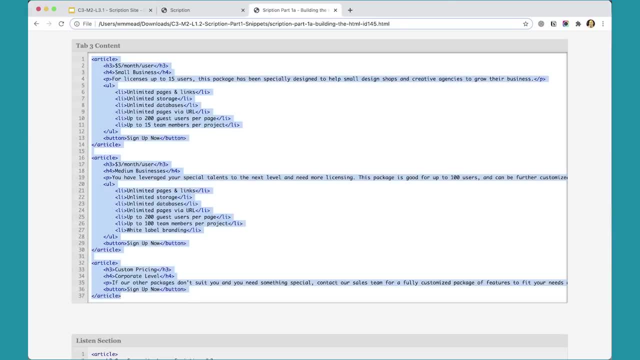 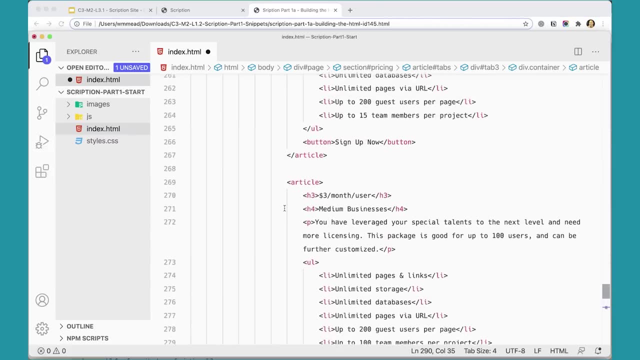 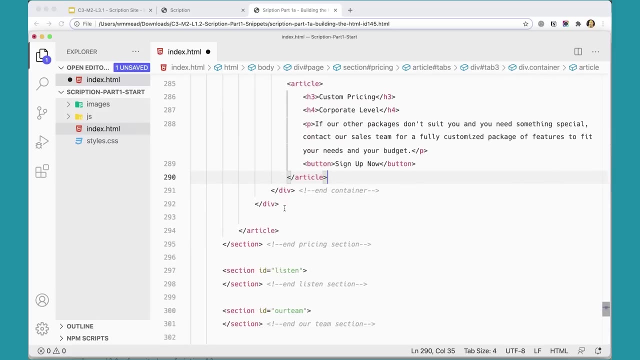 That's a lot of content, And tabs are really efficient at making sure you're not showing too much content at once when they're used properly. So there we go. So we've got all of this stuff in here. We're already up to over 300 lines of code on our HTML file. Okay, great, So we've got all. 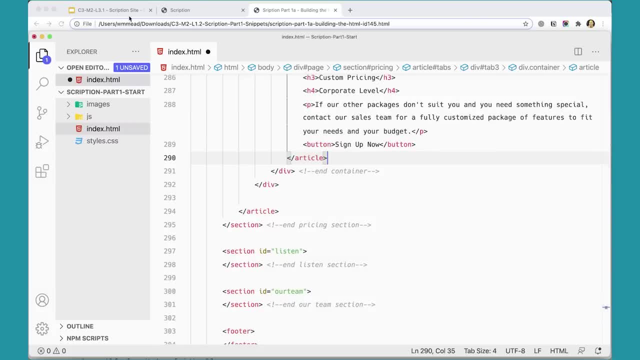 of our tabs in place, And then the next section we need to do, we need to work on, is the tab two content. So we've got all of our tabs in place, And then the next section we need to do is the tab two content. So we've got all of our tabs in place, And then the next section we need to do: 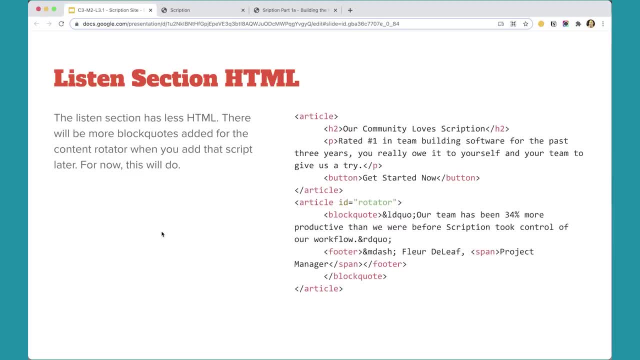 oh, I have the pricing section content here And then the hey listen section or the listen section, And this is going to get a rotator. You can see ID rotator. We're going to rotate block quotes. For right now we've just got one block quote in, But later 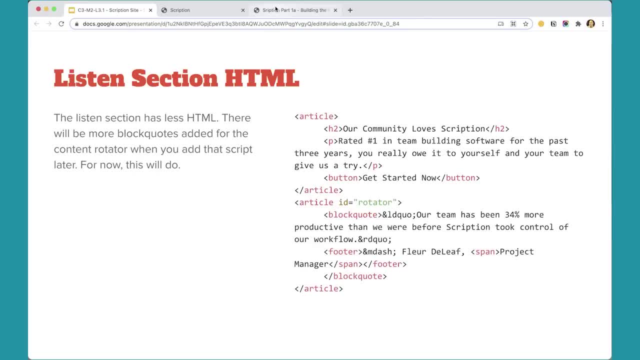 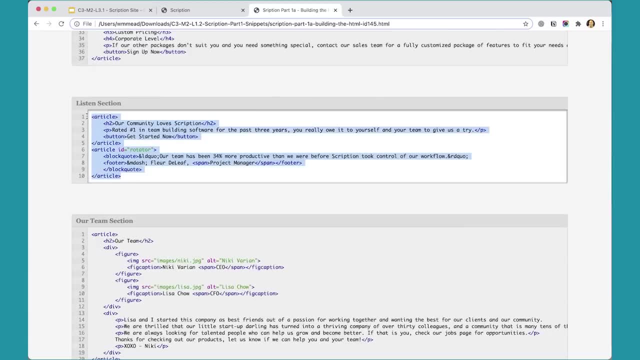 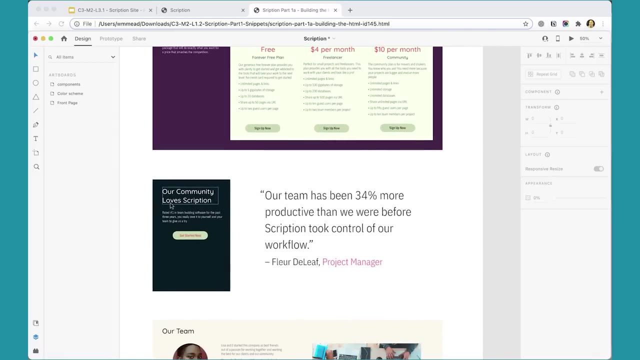 when you make that work, you can add some more block quotes. So let's come over to our snippets. And here's our listen section. And again, just to go over to our design and see what that looks like, That's this section down here. It's going to have this piece and this: 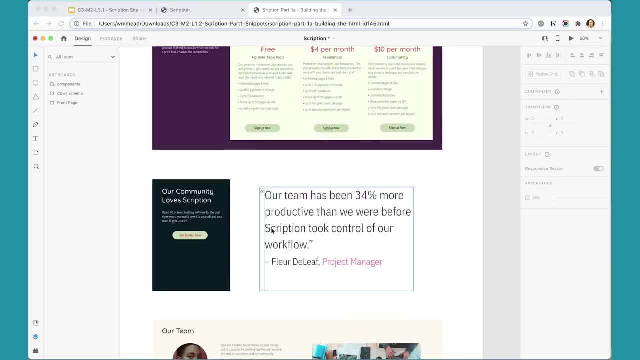 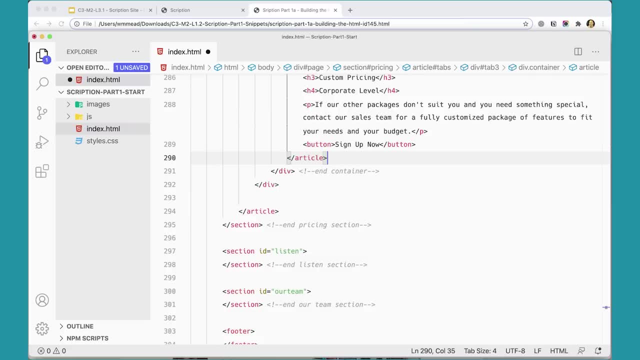 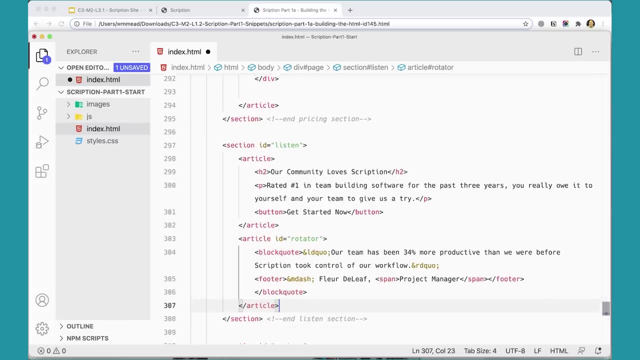 piece of content here which we'll use our rotator, our content rotator, to actually rotate that around. So you'll get lots of practice putting this together. So that's going to go inside this listen section here And then, finally, after that, we have 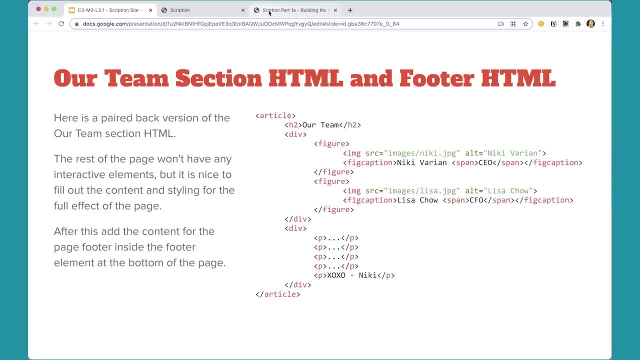 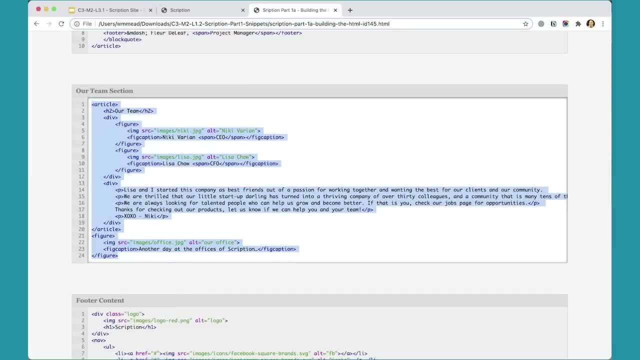 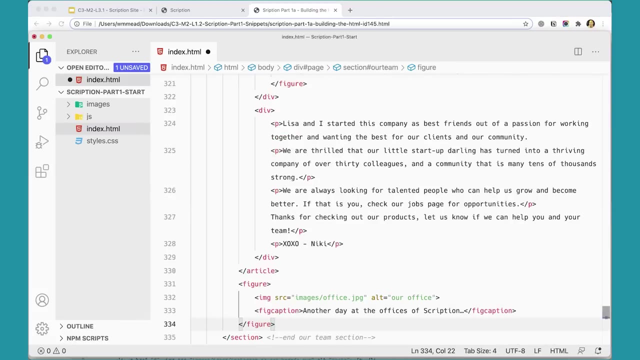 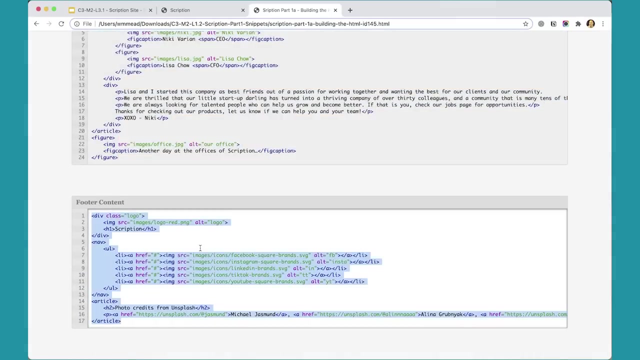 our team, which isn't too long. That's going to be next, Not quite the last thing, but we'll get that next and put that in our team, And then we'll go and get the footer content and copy that and put it into the footer. 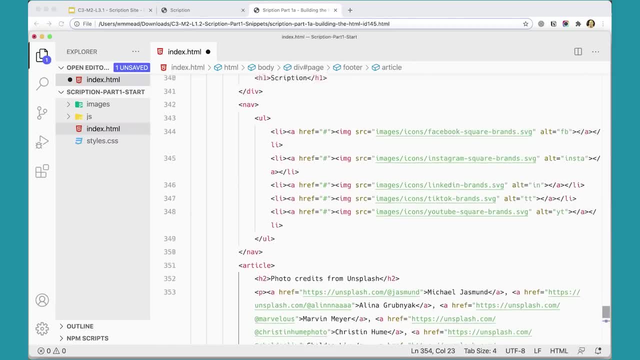 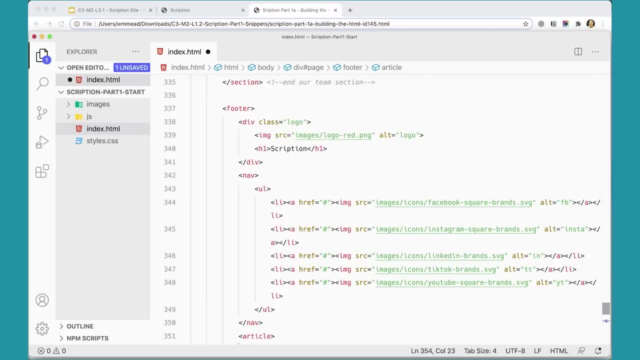 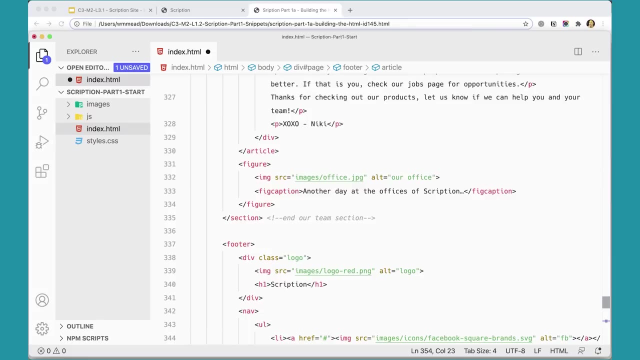 You probably never built an HTML page quite so fast, and it's great to be able to copy and paste this stuff in. but I recommend taking a few minutes to look at how the page is structured, how the content is。。 structured Even better. build that. It's great to be able to repлюс. 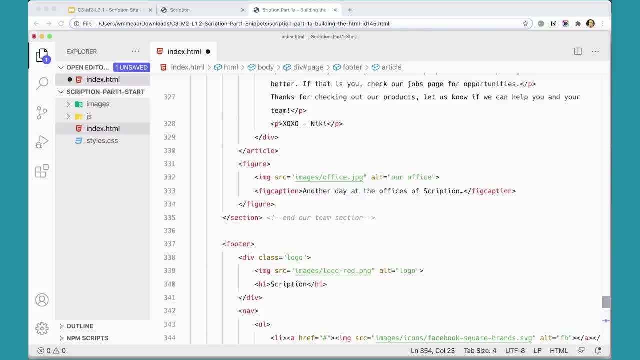 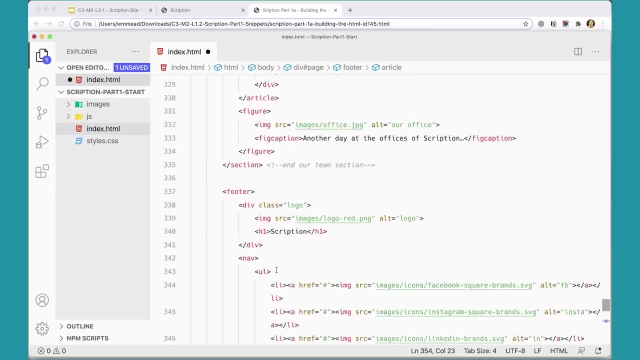 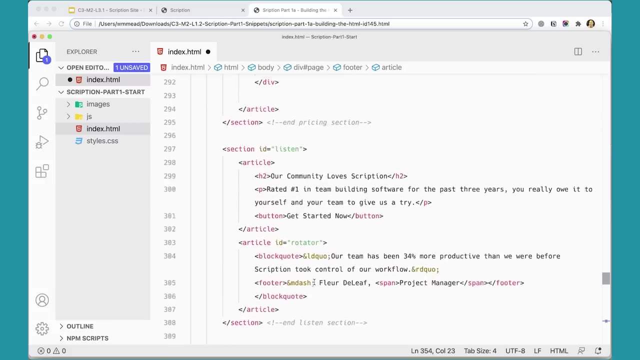 and paste that stuff in, But also make sure that if you're using theese Things that are lists are marked lists, Headings have the correct headings on them, have the correct levels of headings on them, and all of this kind of stuff. 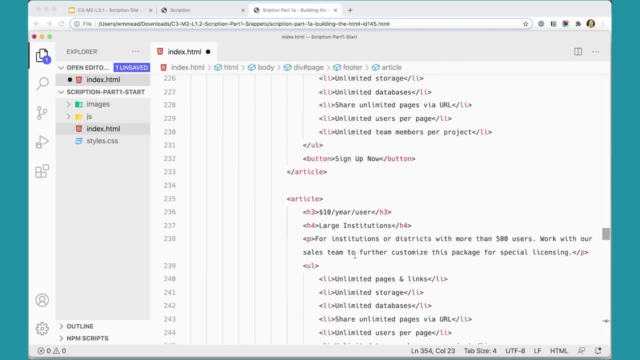 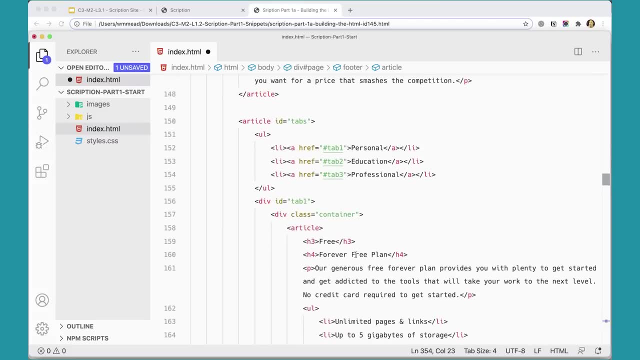 We want to make sure that everything is marked up properly, because Google will be looking at it and scanning it over and using this kind of information to make your page findable. So it's really important to make sure that you're using semantic markup properly. 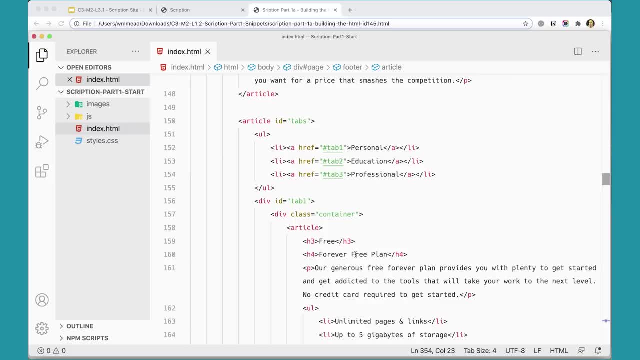 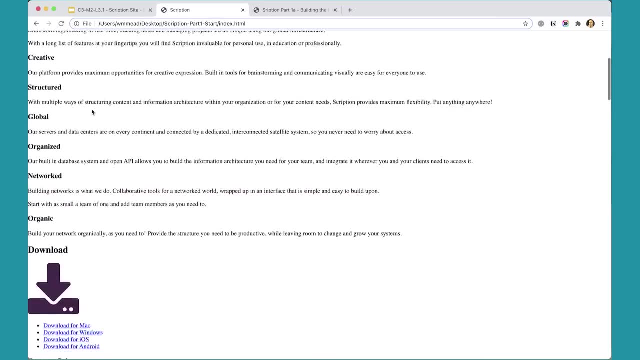 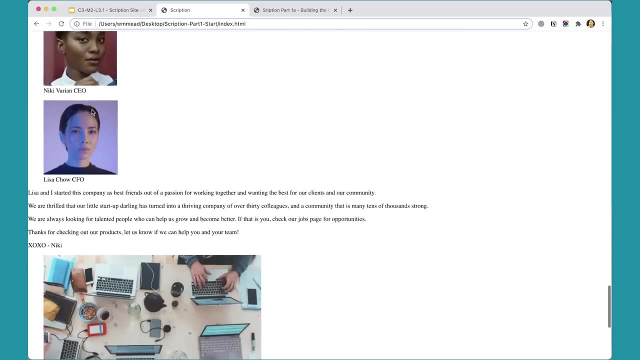 And with that we have all of our HTML in place. If you were to come over and load up the page over here, you would see it doesn't look very good But it's readable Without any styling at all. you could read the page if you had to. 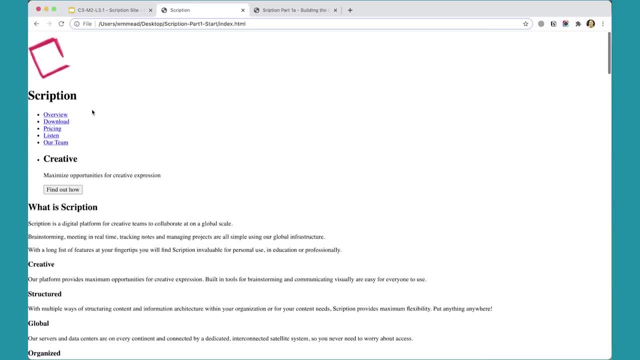 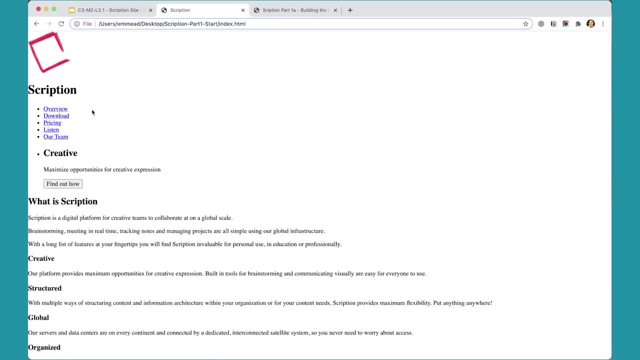 Without any styling at all, And that's kind of. the purpose Of semantic markup is that if for some reason, the styling doesn't work or somebody is working in some real low quality browser, the page is still readable and the information is still accessible. 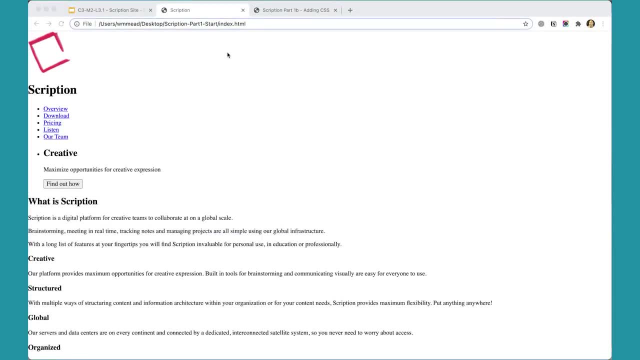 In the last video we finished with the HTML and now we're going to start styling and getting the styling in place, And I have a new set, So you make sure you open this, because we're also going to copy and paste the styling into place. 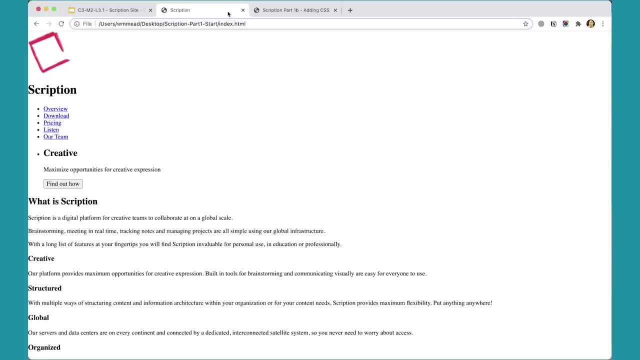 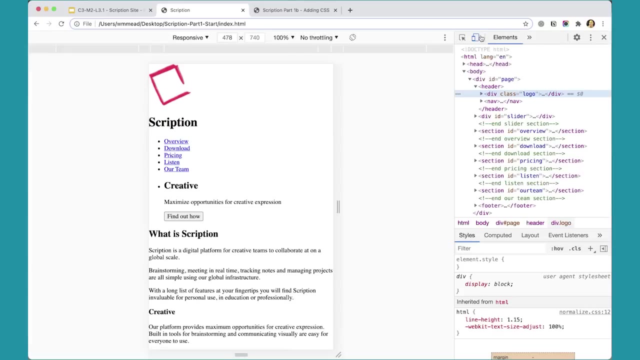 So it goes fairly quickly. But hopefully you got all of this in place And what I recommend you do is we're going to do a mobile first approach. So what I recommend you do is right click on the page and choose inspect And then make sure this little button is toggled on here. 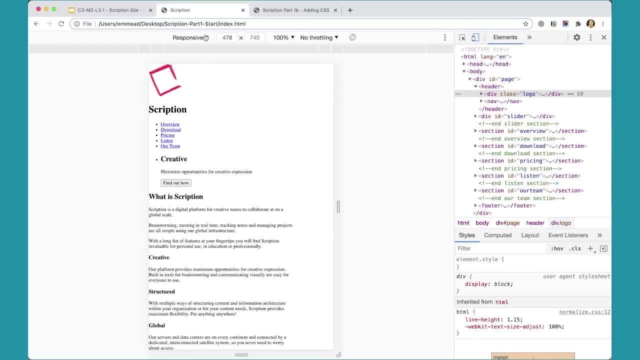 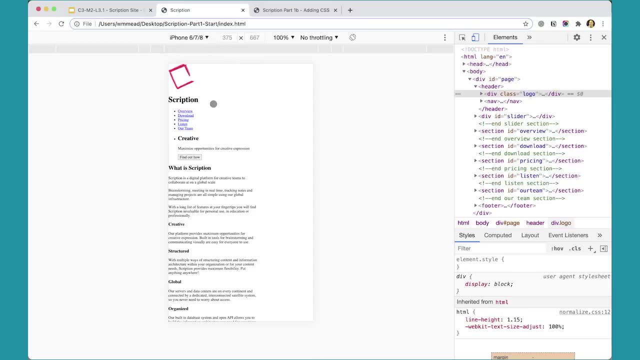 This button here is when it's toggled on, You can actually set a size for your page Here. I'm going to set it to like iPhone six, seven and eight. That seems like a good size to set for to begin with, And yeah, so there we are. 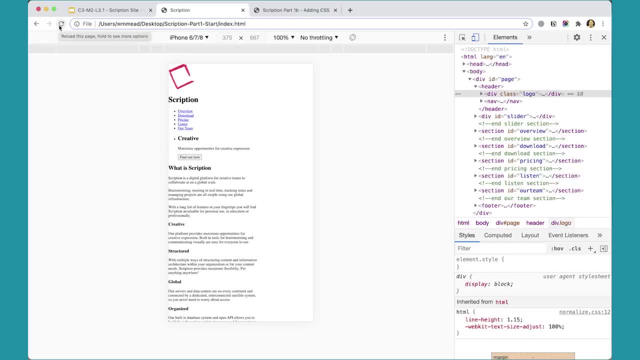 And hopefully that's all working well. If I got the viewport thing set there, Okay, good, So we should be all set with that And from here we We can go over and start working on some styling for the page here. 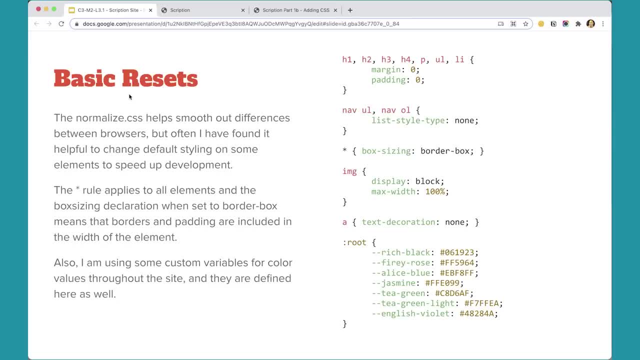 Now I have some initial basic resets. The normalized CSS helps smooth out differences between browsers, but I've often found it helpful to change some default styling on some elements to help speed up development. Removing padding and margin from a bunch of elements helps, removing bullets from unordered lists and ordered lists. 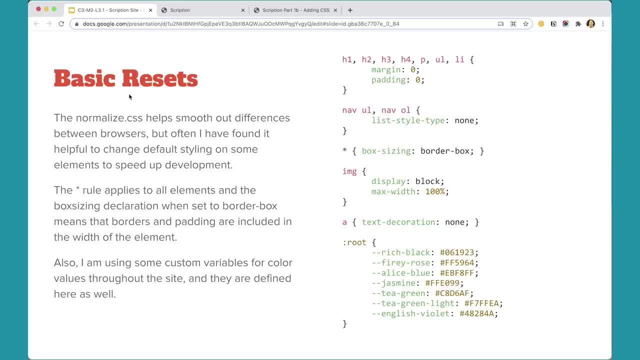 If they happen to be inside of nav. The asterisk on the box sizing means that I'm going to switch everything from using box sizing content box to box sizing border box. If you don't know the difference between those two, I recommend that you look it up and become familiar with it. 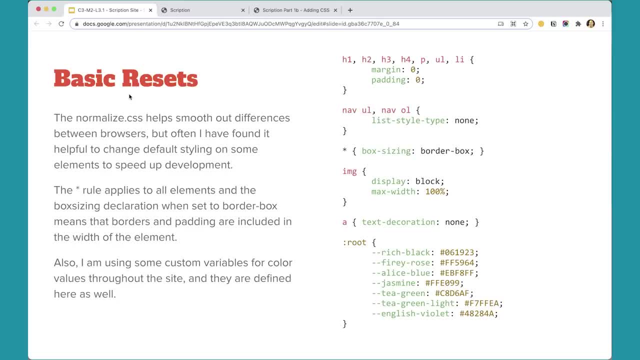 The short answer is that in CSS, when you have the width of an element set- suppose I have a section and I set it to 500 pixels wide, If I had padding, if I had border, if I had margin, I would have a border. 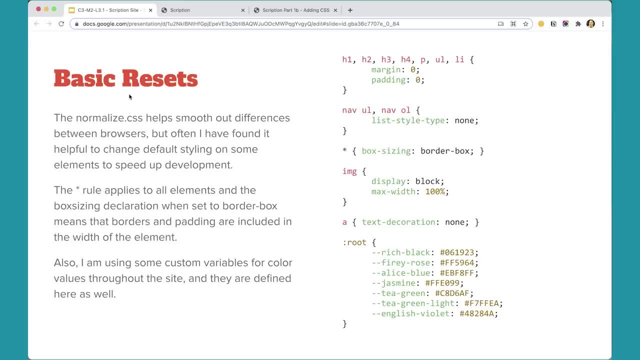 If I had margin I would have a border. It's going to add to the width of that element. The 500 pixels is the width of the content. So when we switch it to box sizing, border box, when I set the width of the element to 500 pixels, that will include the padding and the border, not just the content. 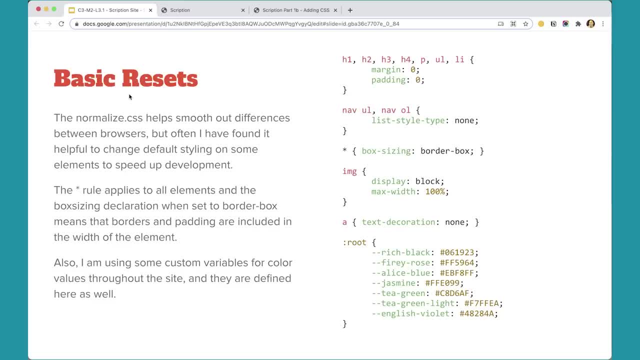 And so that's usually pretty helpful to have set, And we'll just set it that way for everything. For images, I'm going to set the max width on those to 100 percent And I like to set them to display blur And I like to set them to display block. 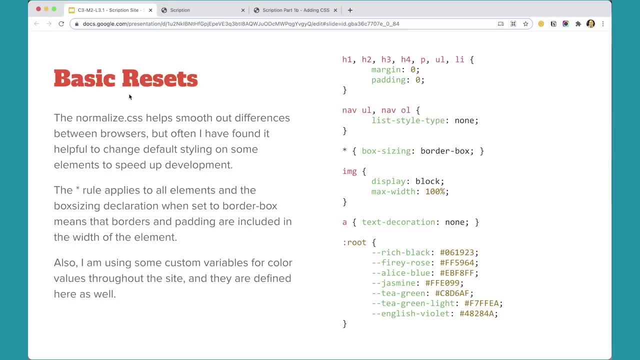 Images by default are inline elements, but we rarely use them inline, So I think it's helpful to set them to display block. I'm also going to get rid of the ugly underlines on links. I don't really like the way they look. 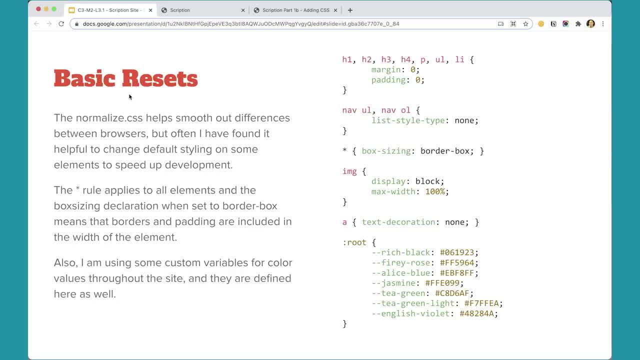 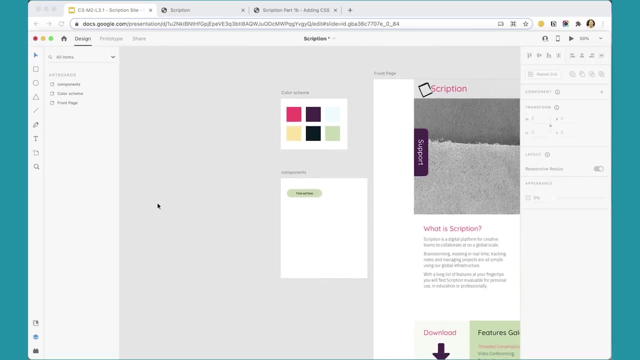 I'll style links differently And I'm using some variables for the colors of the page. So if you wanted to change the colors of the page, you could just change them here once and it will change it throughout the page. If we come over and look at the design here, you can see, if I move up over here, that I've got. this is the color scheme that I'm working with. 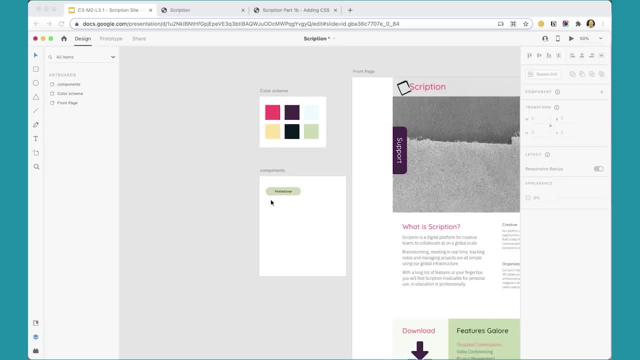 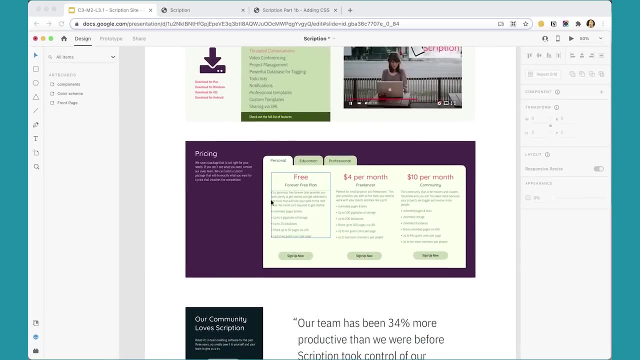 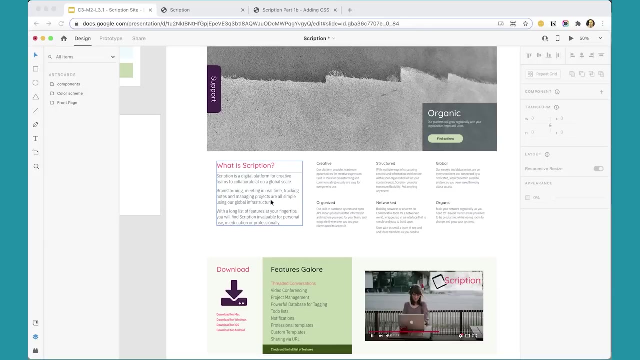 I created a color scheme, So these are the colors that I'm actually working with, to create all of my colors on the page, And it's helpful when you're designing to start with a color scheme And you may not stick with it exactly, but it's helpful to do that. 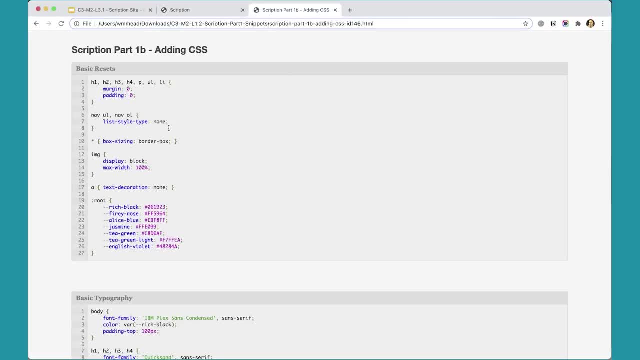 All right, So we can come back here, So we can come over to our snippets here and copy this first snippet, which has all of that basic styling on it, and paste it in over here on our style sheet. So we're going to start working on the style sheet. 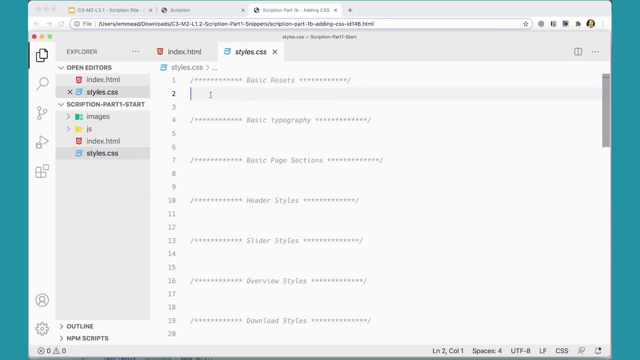 And I'm going to go all the way up to the top and put this stuff into the basics reset section here. Save that And Visual Studio Code. It doesn't like my short end styling for things which drives me nuts, But I have yet to figure out how to get it to not do this. 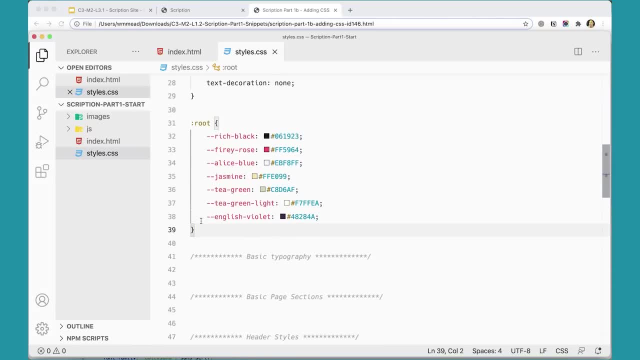 So I really prefer it not to. But that's okay, It's fine. It'll space everything out a little bit further And you know it's always a good idea each step along the way to come back and see how this is affecting the look of our page. 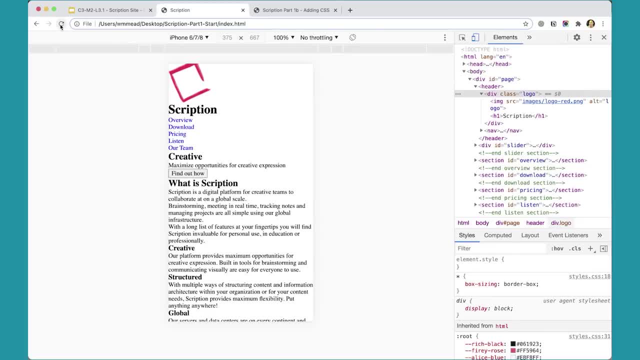 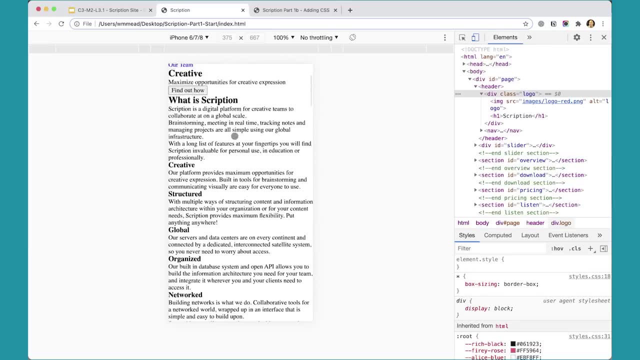 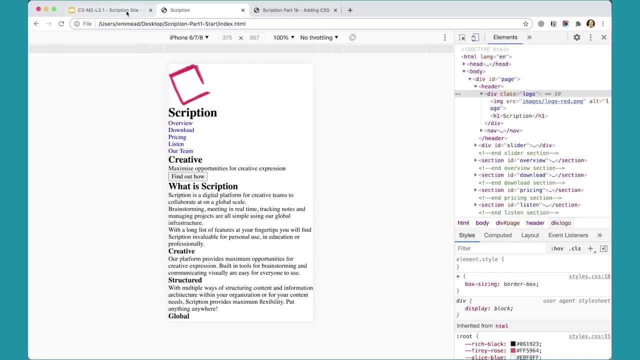 And already it's already kind of affecting the look of our page. It's making it look worse And generally resets do. They'll make your page look worse As you're taking styling out, you're resetting it to a basic and then you're going to add more styling back to make it look better. 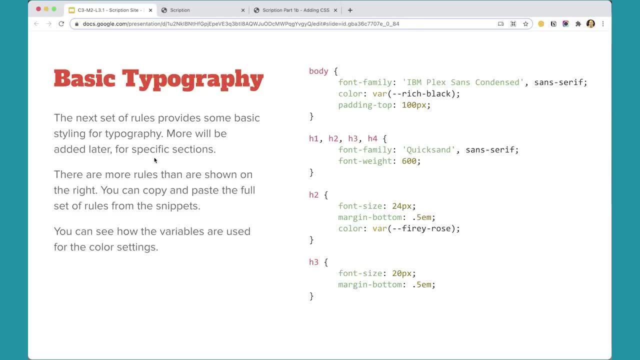 All right, there we are with the resets. That's great. Next we can add some basic typography. Again, I'm using some Google fonts and they're loaded already in the HTML. They're loading from Google. I'm setting some colors, some sizes and that kind of stuff. 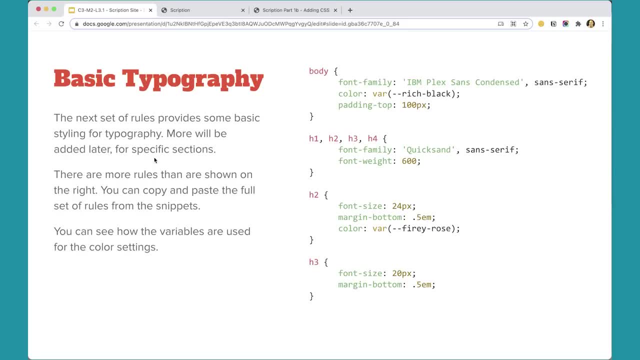 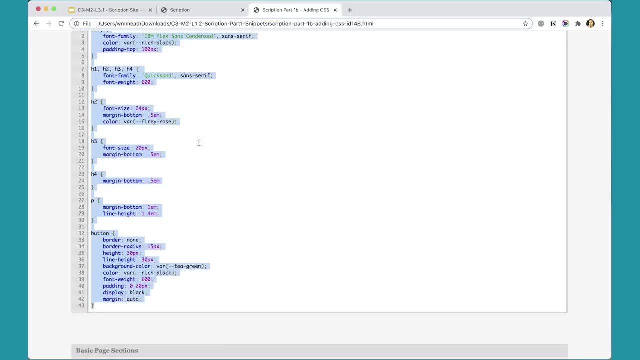 And you'll see that this will quickly start to bring some life and breathe some life back into the page as we add this stuff back in. So let's go over to our snippets and add these rules here, And there's more than what I showed on the page. 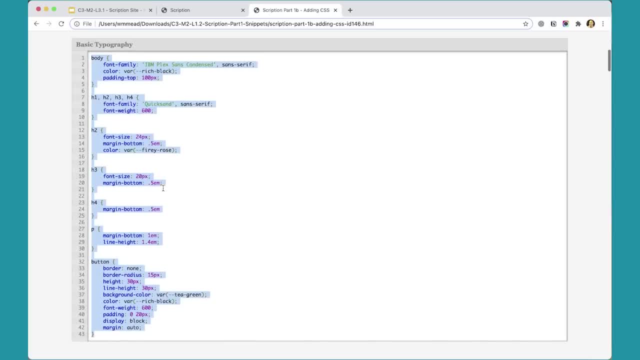 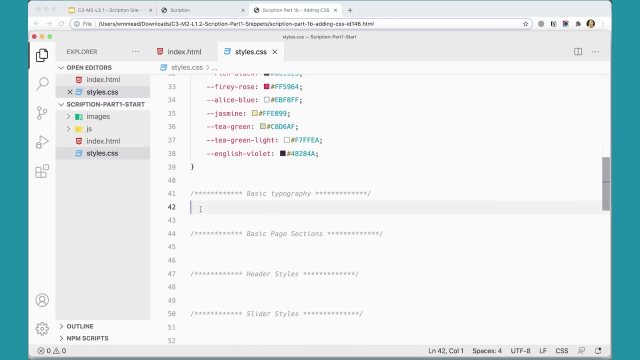 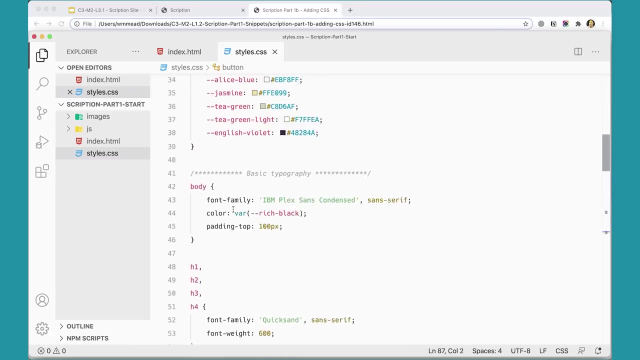 This rules for the footer and for the button as well, So we'll add those in under basic typography, And I do like to do things in this order, where I sort of set some basic settings for the page, basic resets, typography and maybe some basic page section stuff that's going to get inherited across the entire page. 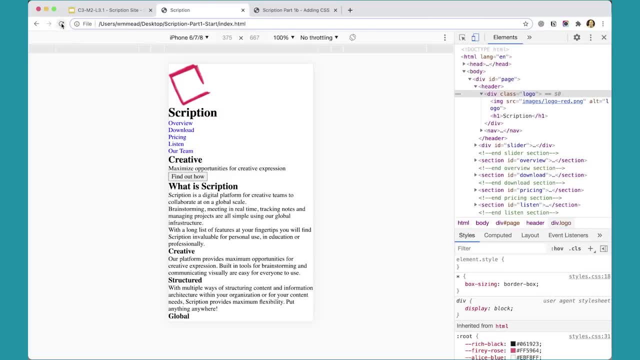 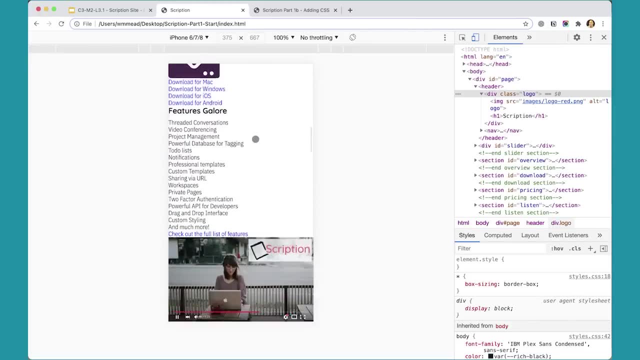 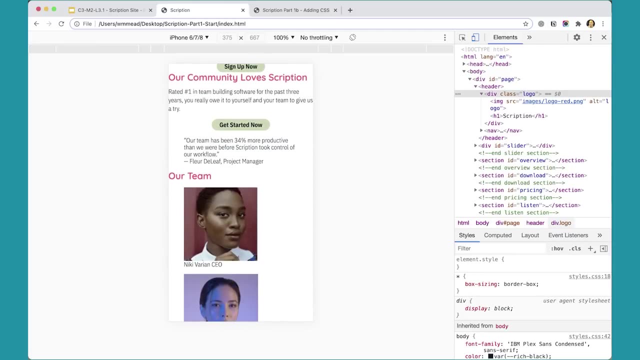 Let's go. Let's go take a look at what that looks like with those rules applied. Boom, Already starting to look a little bit better. once we get a font in there and some stuff working along and going along, That's great, All right. 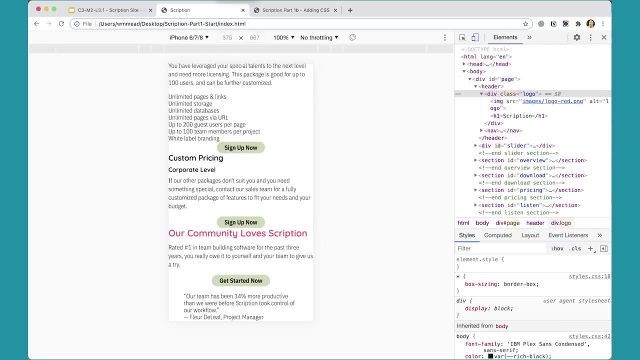 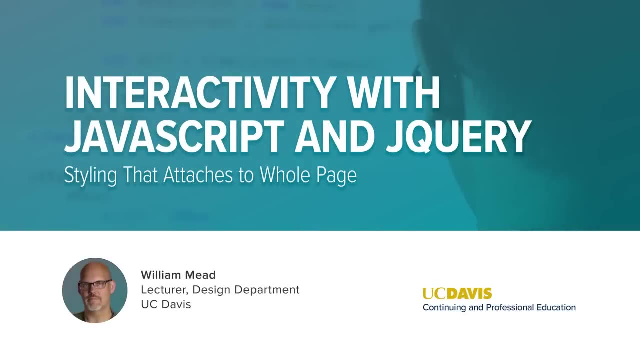 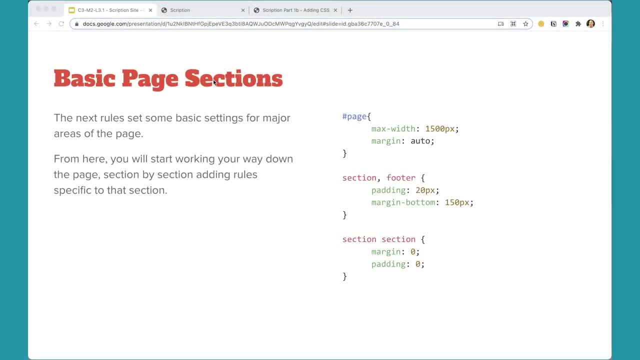 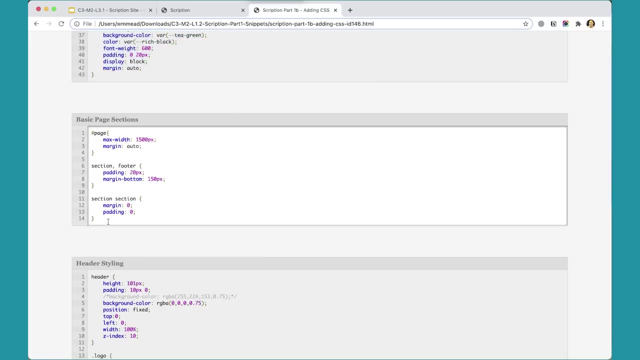 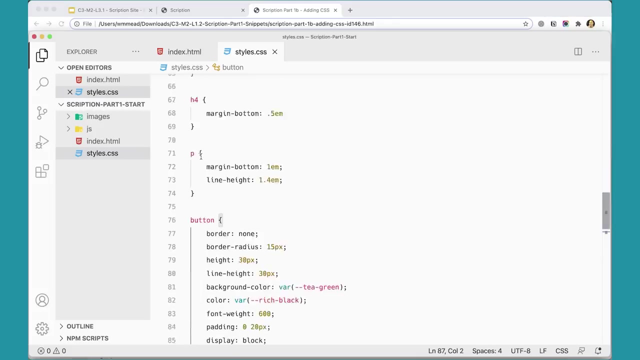 We'll continue with the styling in the next video. Next, we'll apply some styling that will attach to the whole page And there's just a few rules here, but they'll actually make quite a big difference. So let's go over and grab these three rules, paste them on our style sheet here inside the basic sections section. 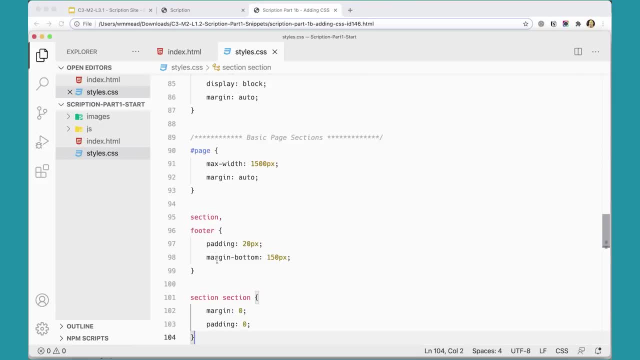 And you'll see, just with these little bit of rules over here, it's going to make a lot of sense. So let's go ahead and do that. It's going to make a big difference. Currently we've got no padding here. 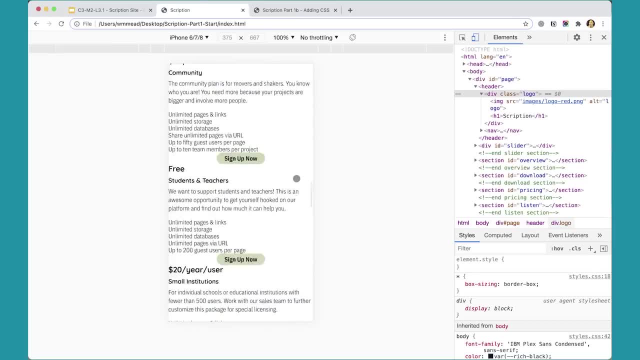 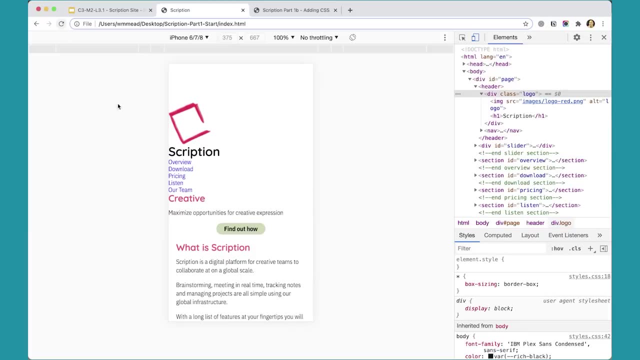 It's running right up against the edge. It's kind of a mess. It doesn't look that great yet, But I'm going to scroll up to the top here And if I refresh, you'll see immediately. we're starting to get some spacing between the sections a little bit more. 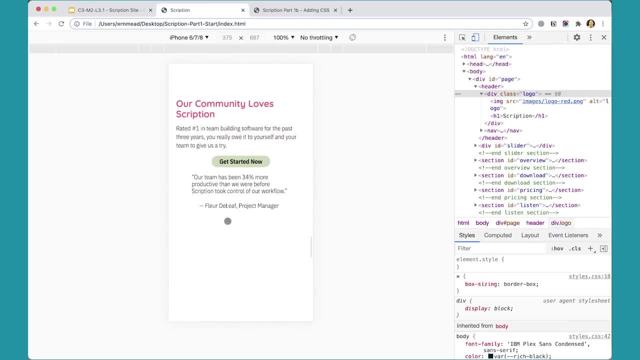 It's getting a little bit better, a little bit more readable, Coming along. Now. this is going to be more concise, But it's going to make a big difference. It's going to make a big difference. It's going to make a big difference. 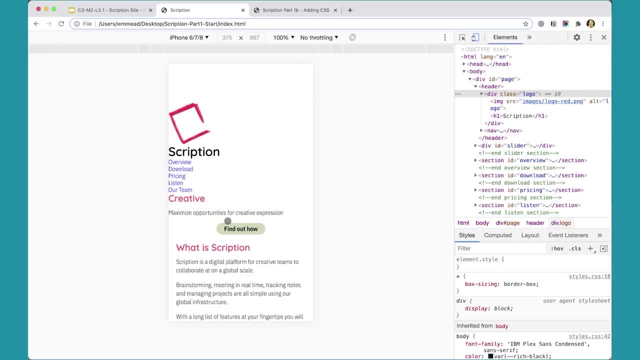 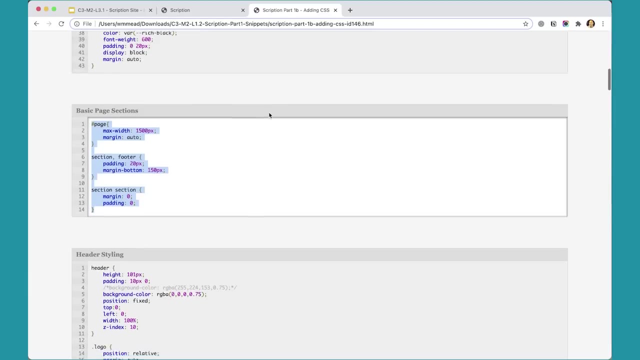 down the page, starting with these basic sections and as stuff further down the page is inherits, then you need fewer and fewer rules. as you go down the page you'll see is it sort of works out that way. headers are always a pain in the neck. they always have a lot of styling in. 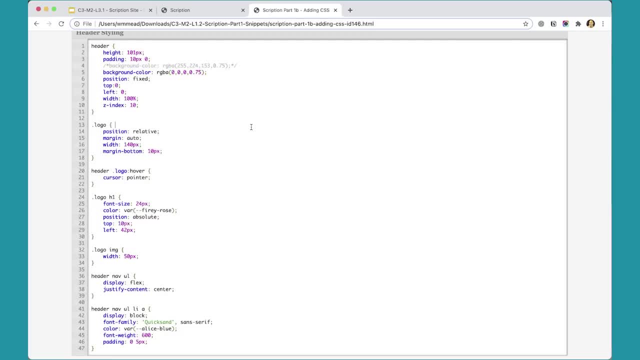 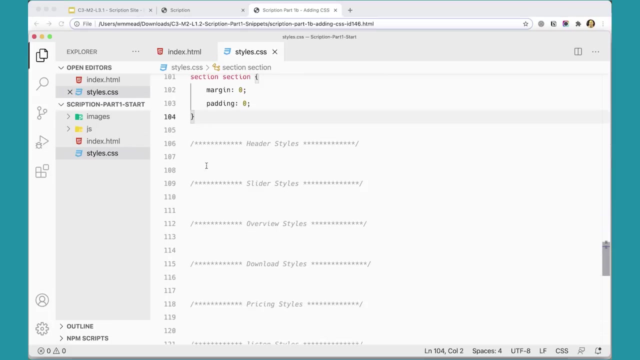 them to kind of get things to look right, and so I'm going to copy all of this stuff and I'm going to go ahead and paste that in in the header. they had a section here. there's a lot to look at in these header style, so it's worth spending a few. 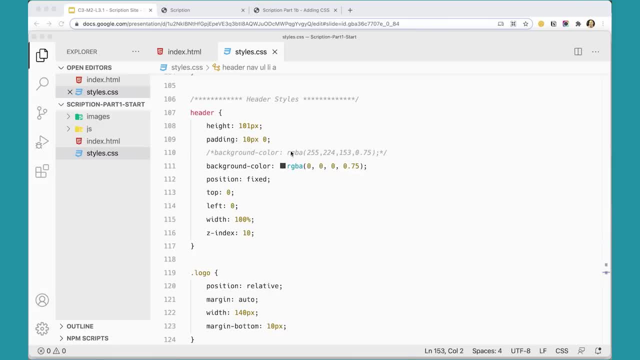 minutes on this. I changed my background color again because I don't have a lot of font options. so I changed my background color again because I don't have a lot of font options for that- for my header here- to a gray. but you could try a different background color. this is: 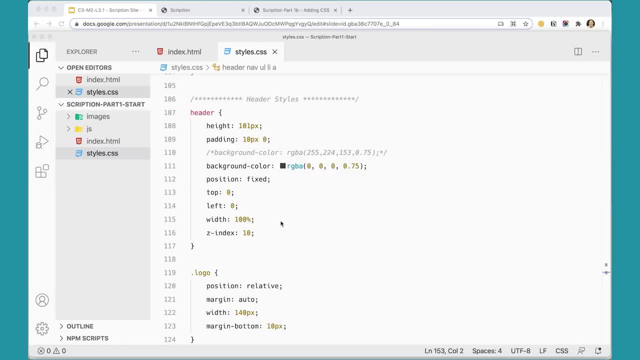 one of my other colors. um, with some transparency. the 0.75 gives it a little bit of transparency, but you could uncomment this out if you wanted to see how it looks. um, the header is going to be set to position fixed so that the header stays up at the top of the page, no matter what, as you scroll. 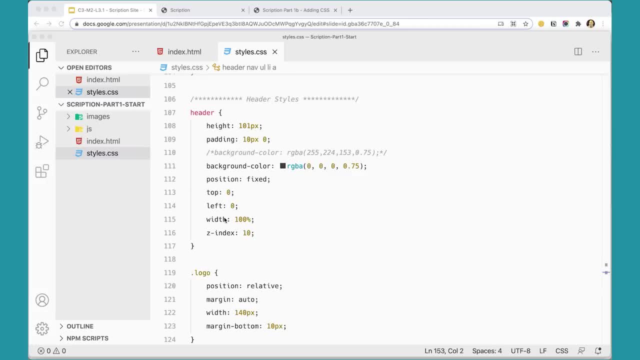 down the page and i'm setting the top zero and left zero and then with the hundred percent and i'm making sure it stays on top of the z index set to 10.. the logo is going to be set to position relative because i'm going to do some absolute positioning for the h1 inside that logo down there. 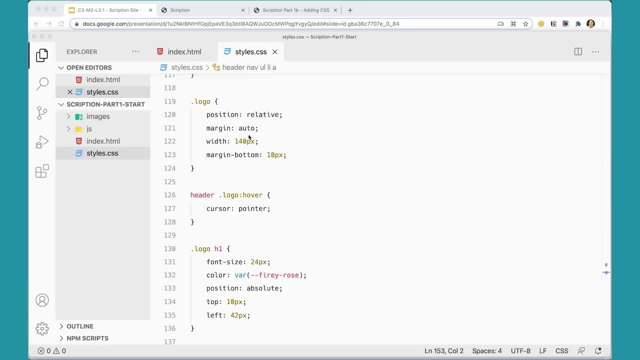 so that's such a relative positioning margin. auto is going to center that, give it a width and set the margin on the bottom. i have the. when you hover over the logo, it's going to turn the pointer to a cursor because ultimately that's going to be a link, something that we can click on, and it's going to activate a smooth 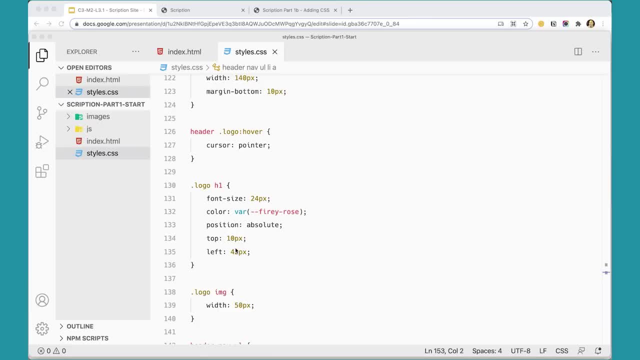 scroll effect that you'll put in later when you're completing the interactive challenges part of this lesson, but you can see basically everything's kind of coming into place here. i've got the the rules for the navigation in here. we're displaying it as flex. flex is a display method that allows you to get things to line up next to. 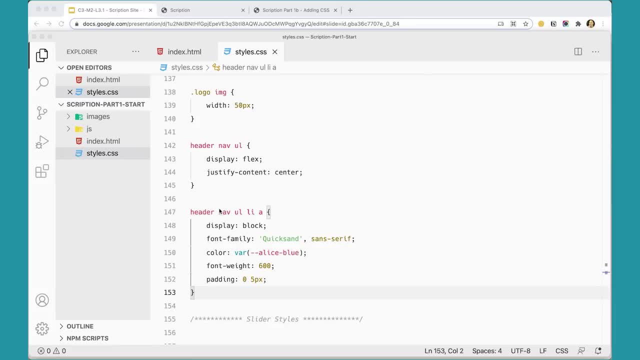 each other in a row, which is what we want for our navigation, and then the anchor tags are set to display block. and that's because anchor tags by default are inline elements and usually in navigation you want them to be block elements. and then i'm setting my colors and my font size. 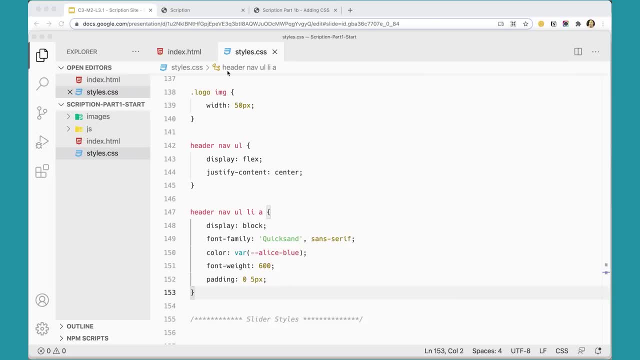 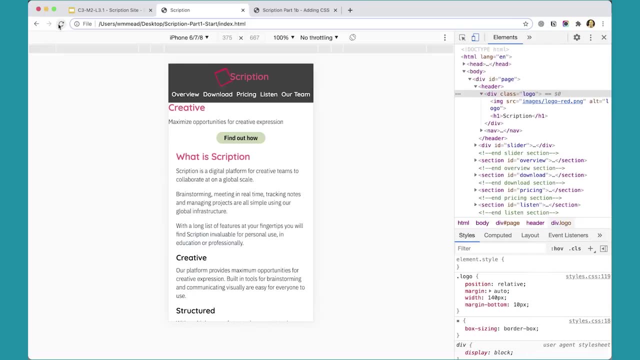 and that kind of fun stuff. so with all that in place, we should go over and take a look and see what this magic does to the header, header of our, of our page here. boom, look at that. all that styling got that all into place. so the navigation could maybe be a little bit better for mobile. 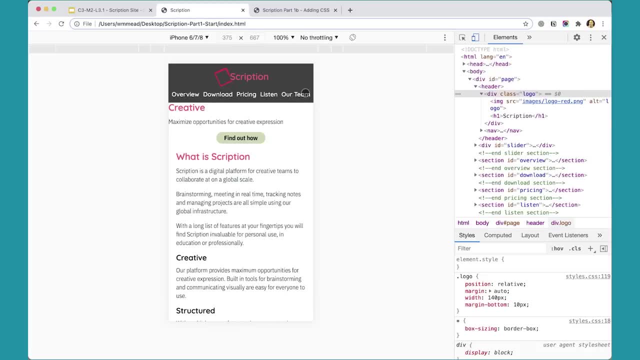 i'm kind of squeezing it all in here. you could replace it and put a hamburger menu and have a drop down menu, but that's a lot more work and i wanted to make the a little bit. otherwise it was going to be a lot of work if i added that for you. 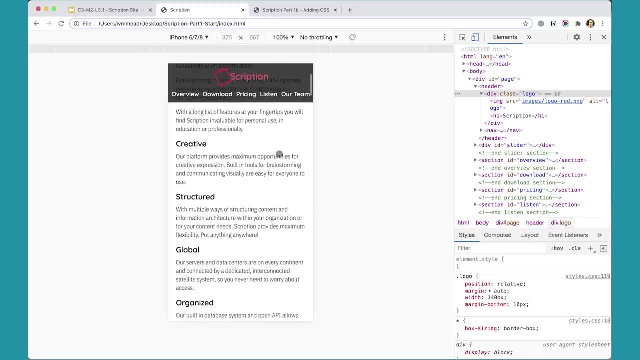 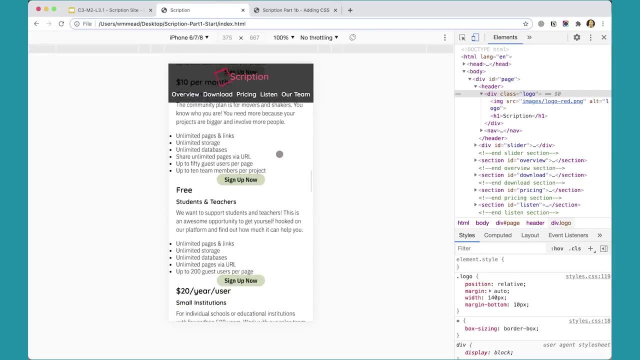 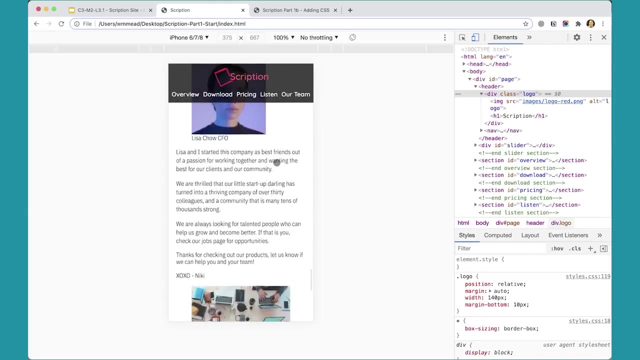 and i. i didn't want to do that, but you'll notice, now the header is fixed. so the header will stay there as i scroll down the page and if you wanted to try the greenish background, you could put that in if you wanted to. i kind of like the gray in the end. i kind of liked it that way. all right, so the header's in place. 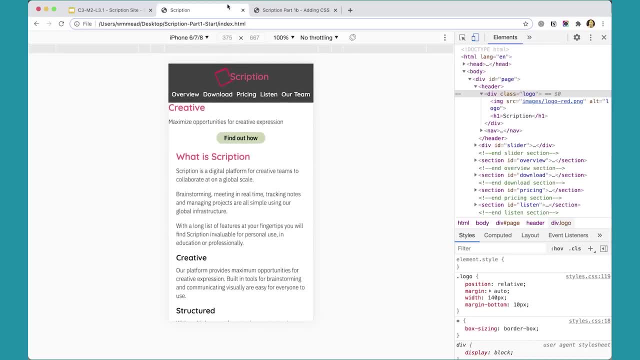 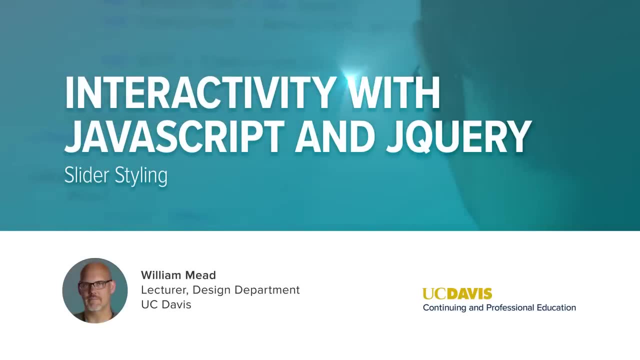 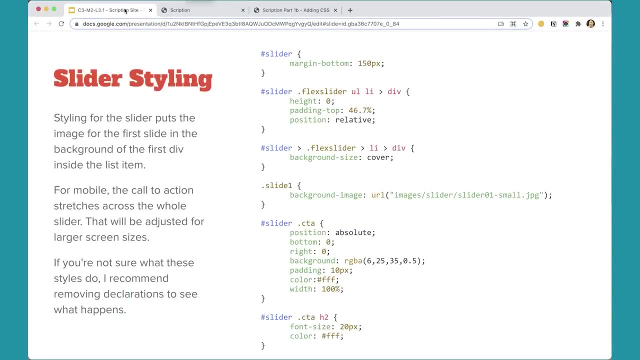 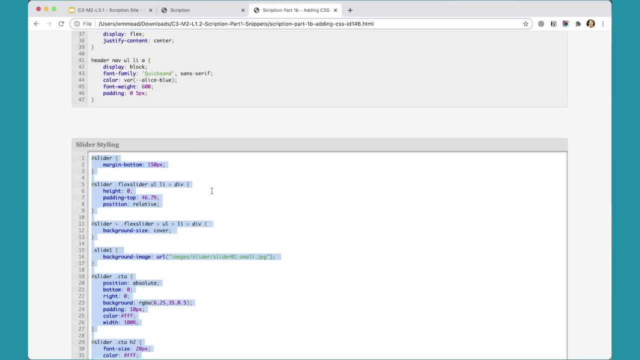 and we're ready to see what we need to do for the next section, continuing with our styling, we'll add some styling for the slider and these styles again are on the snippets and it puts the image for the slider in the background of this element. so let's go ahead, come down here and add this. i'm just going to copy all of this. select it all. copy. 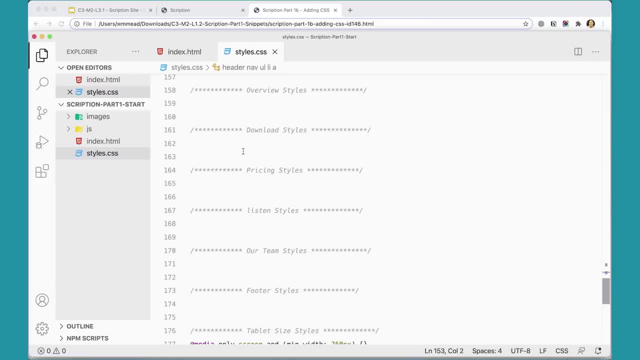 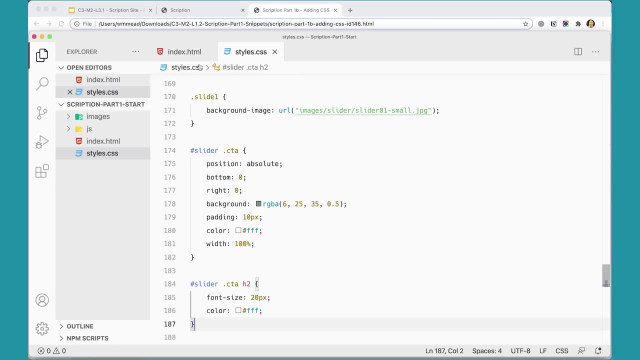 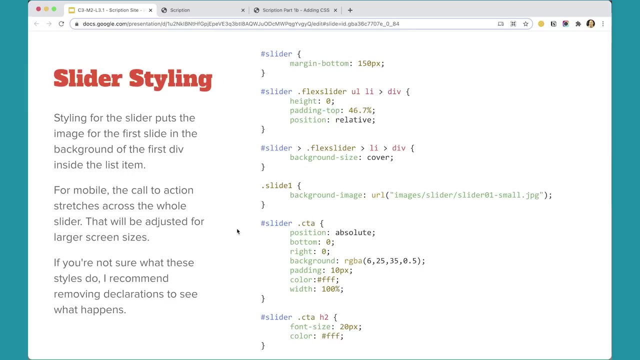 and then come over and add this into the section for the slider here- and there's a lot going on here and if you're not that familiar with css, i recommend poking around with this. what happens if you remove some of these declarations and see how it looks? see. 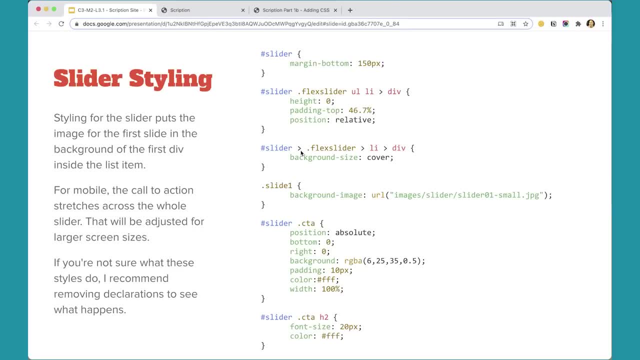 how it changes it. the angle brackets here indicate that i'm applying this to the direct child and this makes sure that if i that, um, if i have another div that's further down the the chain, that it doesn't get that uh styling attached to it. um, but the best thing to do if 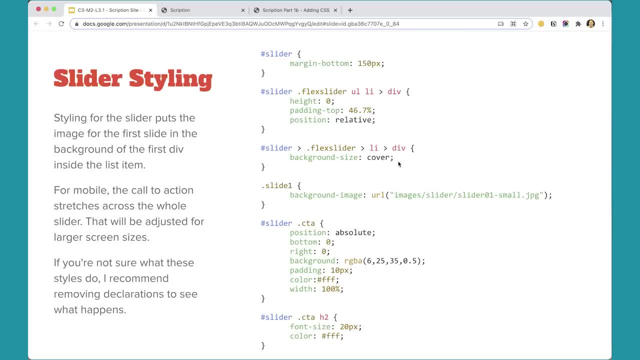 you're not really sure about how this is working is to sort of mess around with it, play around with the settings. even if you screw it up entirely, you can just delete it and then paste it back in again from the um, from the snippets. so don't worry about that um, we'll have some stand-by as we go down again. so i'm just going to go ahead and go around into the olsun settings and then, uh, then we'll raise them to our inbox and make sure that it's actually located on the css template, and i just want to take a look. do i want? 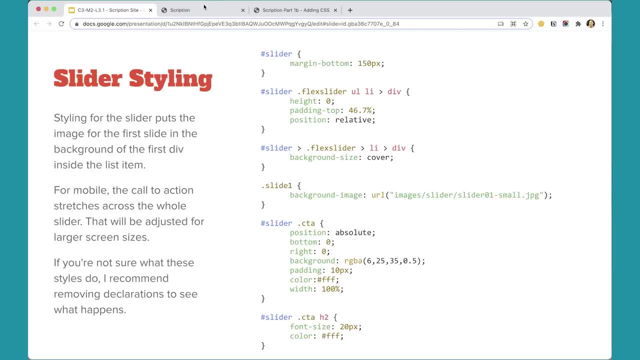 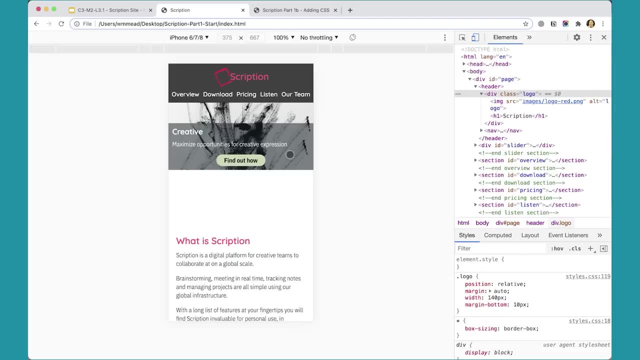 snippets, So don't worry about messing it up. All right, with that in place, let's go see if our slider is displaying properly. And there we have it. And for the mobile version, we're going to have this call to action sort of stretch across the entire slide And it'll look better for the. 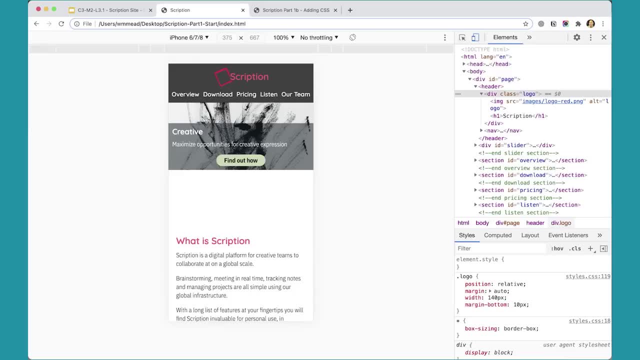 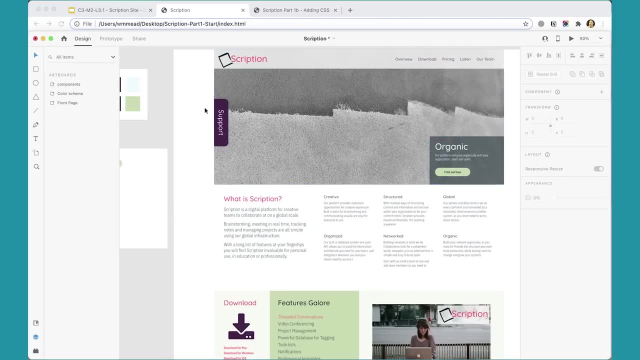 desktop version Because, as you saw over here, it's going to look a little bit different When we get to desktop. it's going to look like this instead- And I've left off this thing. I actually decided to put that in- But it's going to look like this with our call to action here: 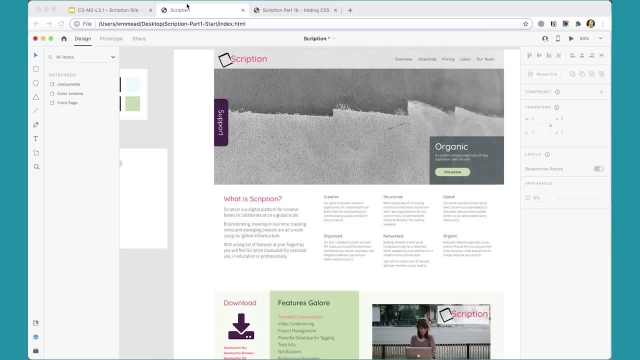 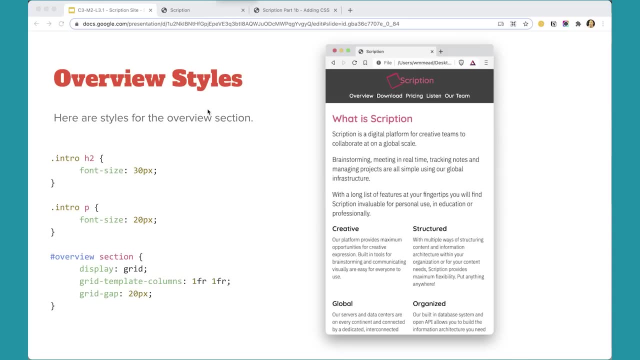 instead. Okay, so we've got that in place And we're ready to go on to the next part. We don't need to do much for the overview settings, because a lot of it is set nicely already by the styles we've already added. 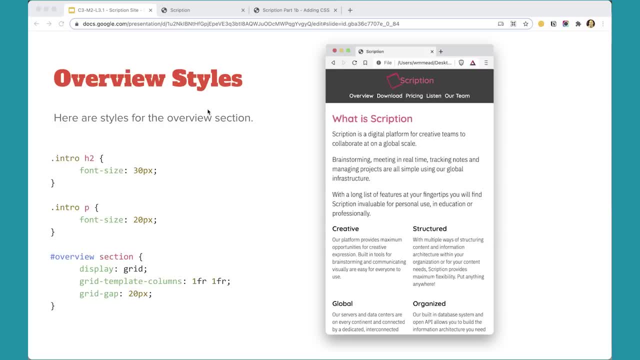 So this is what I meant by, as you go down the page, you need to do less styling, because a lot of things get inherited. So we just need a few rules to kind of sort out some of these things and set the overview section to display as a grid so that it looks right there. So let's go ahead. 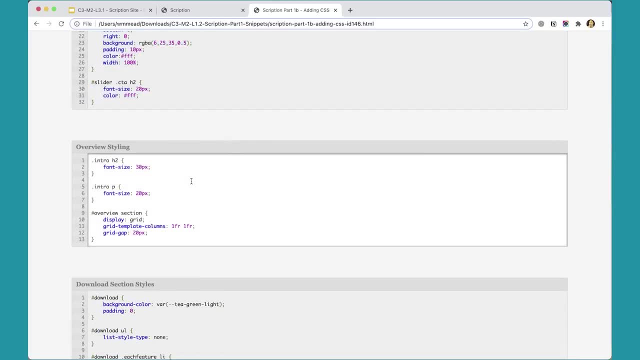 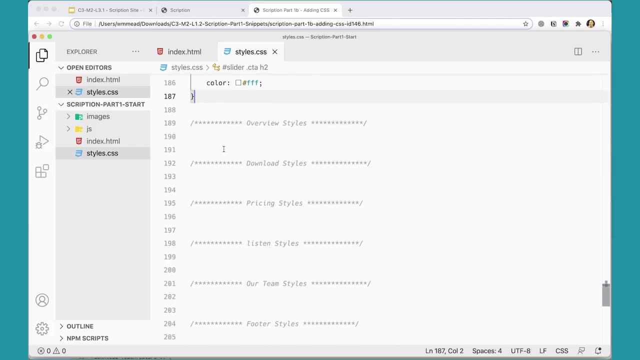 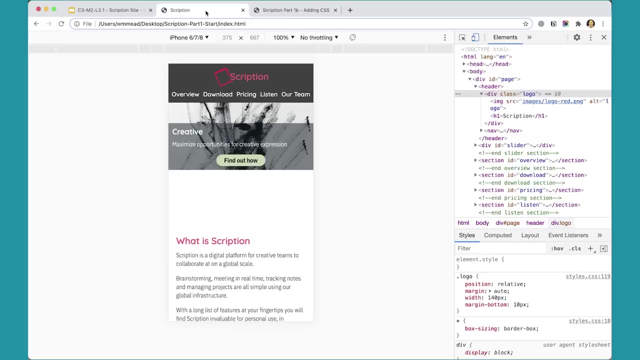 and add these rules for the overview section. Just a few of them here. We just need to stick in over here Inside the overview. I'm going to save that And then when we come back and refresh the page, we've got what description and we've got kind of an overview here. 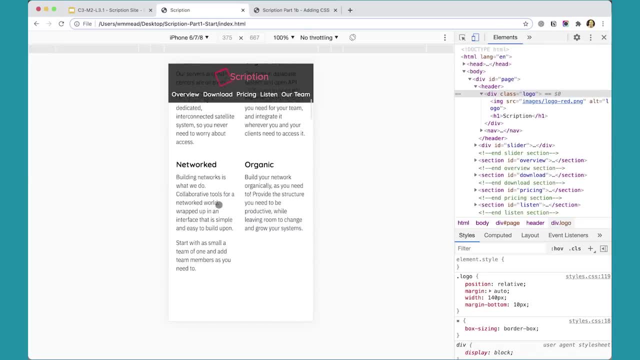 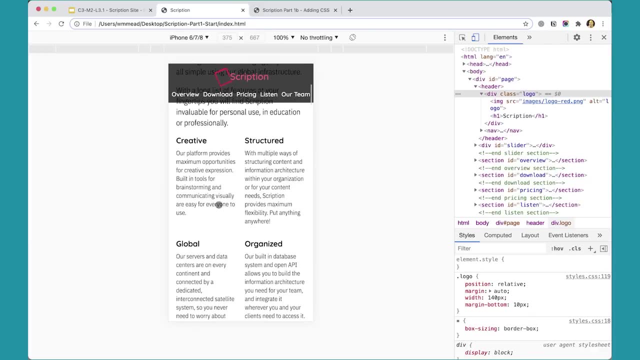 with our columns of stuff And it looks really good. It looks really nice. You can imagine seeing this on your phone. It should look pretty nice. And again, we're doing the mobile first because we'll be adding the desktop view in later, And then next we've got to look at the desktop. the download section. 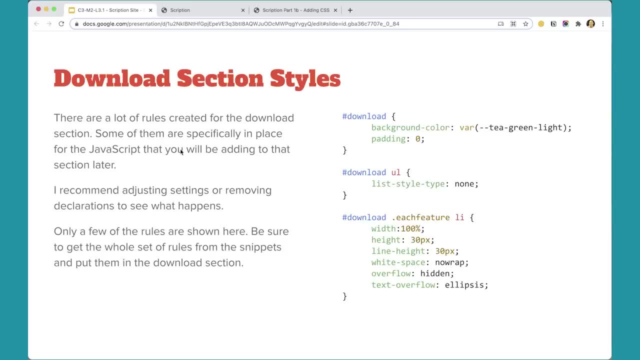 Download styles. let's add those. There are a lot of rules for the download section. Some of these are specifically in place because of the JavaScript you'll be adding later, And again I recommend adjusting The settings are removing declarations- to see what happens. 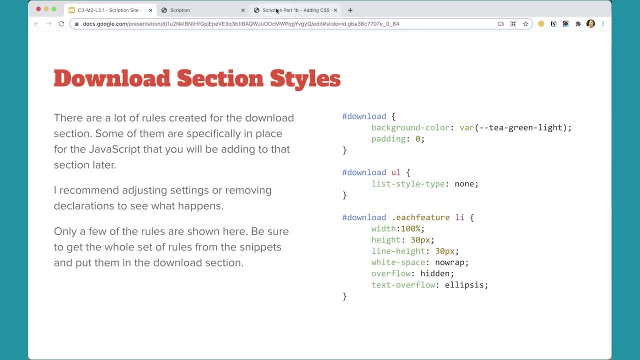 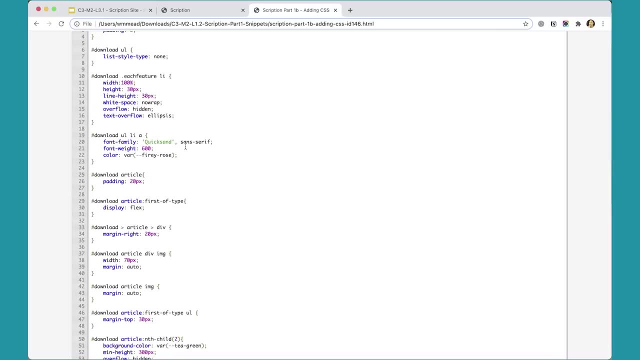 Only a few of the rules are shown over here, but I've got a lot more on here. There's a whole big chunk for the download section. That's a lot. Let's just grab it all And again, the best thing to do is to kind of mess with it and see what happens if you mess around with it And if you. 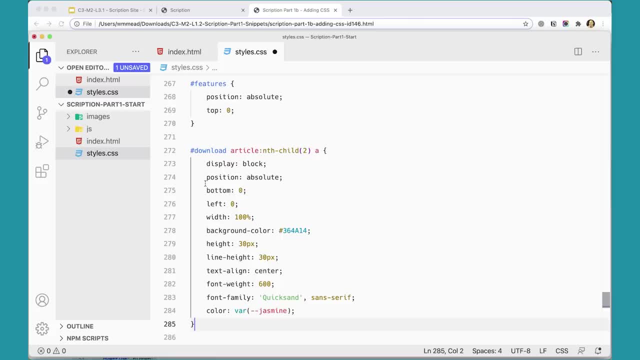 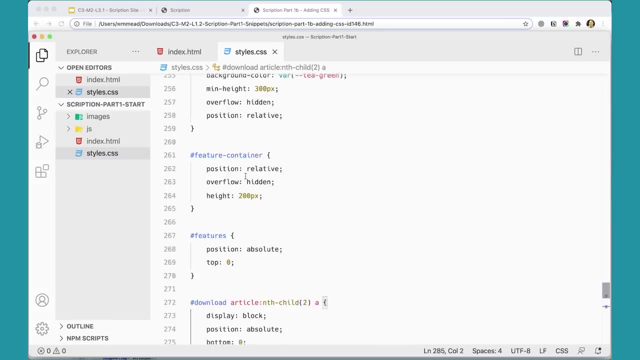 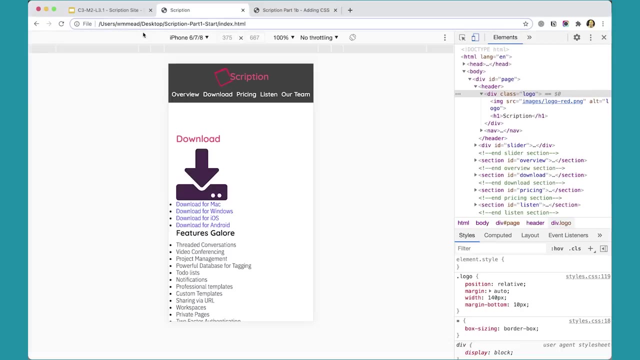 screw it up. you can always paste it back in again. It's not a big deal, So we'll put that in. I'm not going to go through and describe all of these, but they're all in here. Let's go take a look and see what that did to our page. 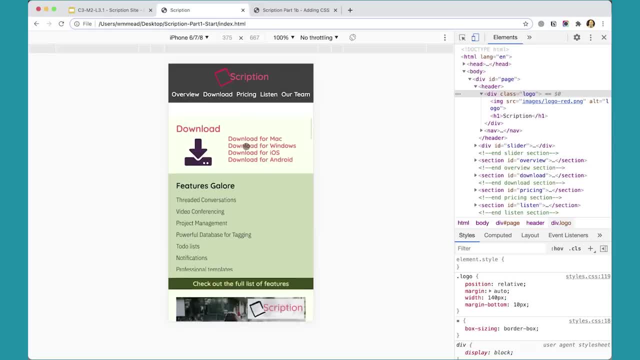 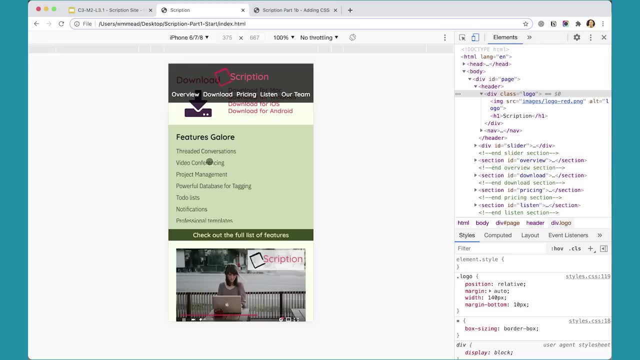 Download section. It looks pretty nice for mobile like this. This thing here is going to be an element- I'll show you the finished version- that sort of animates and moves these things up and down or moves the bottom. So this thing right here I'm going to move the bottom line up and slightly move the fingers on the right side. 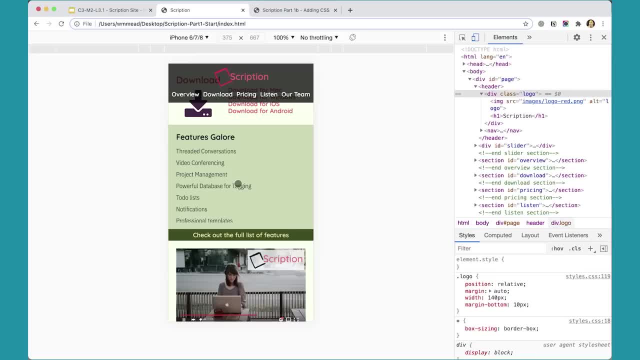 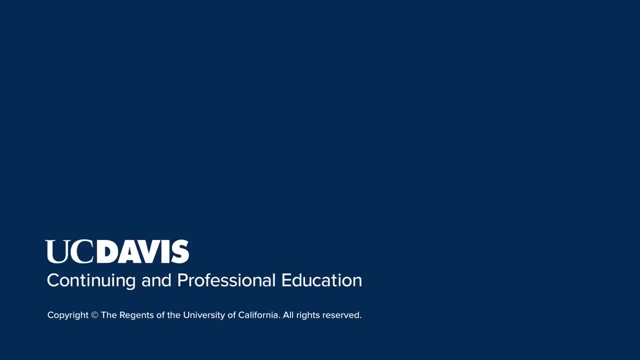 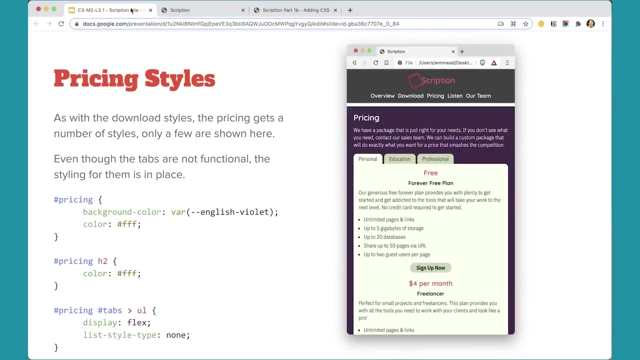 or moves them up into place and highlights them as they go by, And you'll be adding that script. You'll have a challenge to add that script on your own in a future lesson here. Okay, great, We're coming along. We're going to continue adding styling to our page. 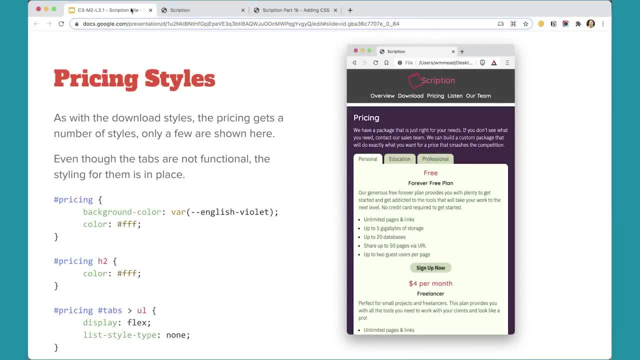 and the next section is the pricing styles And that's going to set us up to get our tabs working the way we need them to work. when we add the tabbed script later, You'll be able to add that later and make that work. 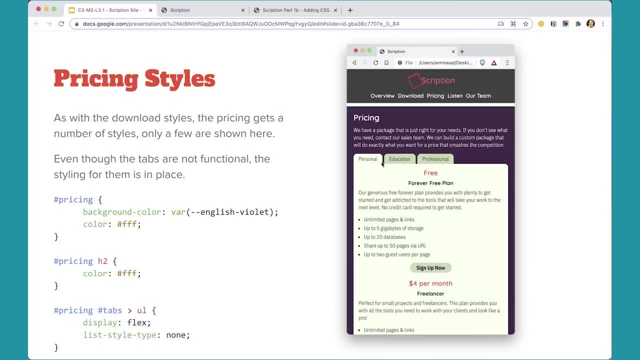 So most of that content is going to be hidden because we're only showing the first tab and the other tabs are going to be set to display none. So there's only a few of the rules shown here, but there's a lot more over here on the snippets down here. pricing section styles. 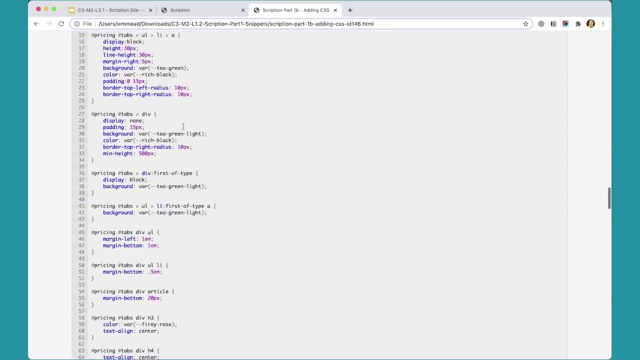 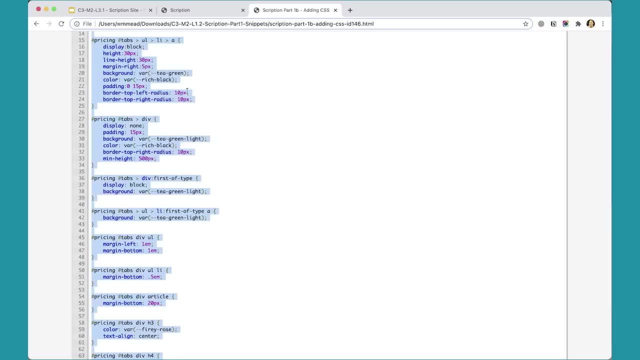 You can see there's a big old chunk. And again, if you're not sure what these do, I recommend playing around with them and inspecting your page. Take some out, See what happens, Change the values, Mess around with it. 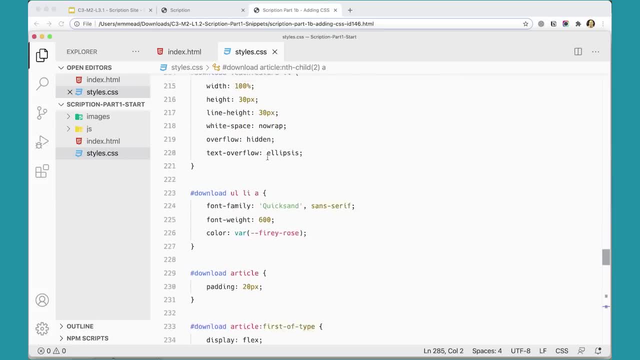 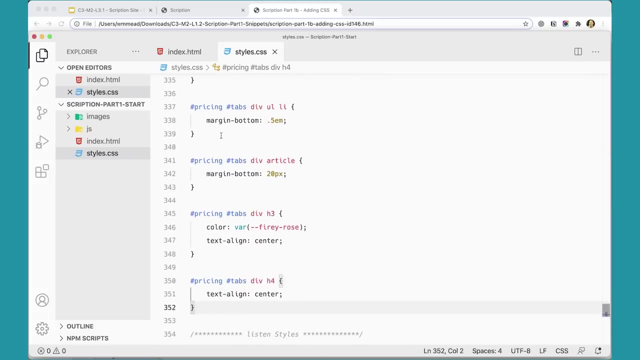 It doesn't matter if you screw it up, It's totally fine. So I'm going to go ahead and add those here under the pricing style section And you'll see Once we get that in and save it and then come back here and refresh the page and scroll down to the pricing section. 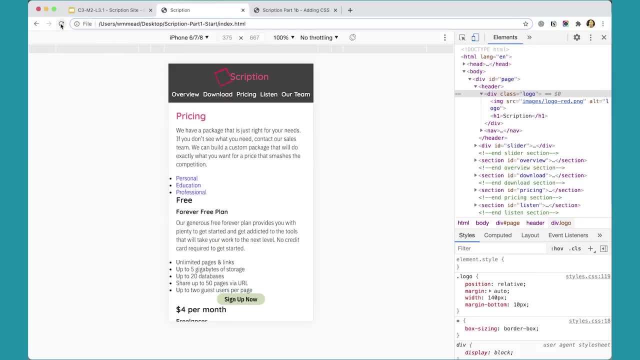 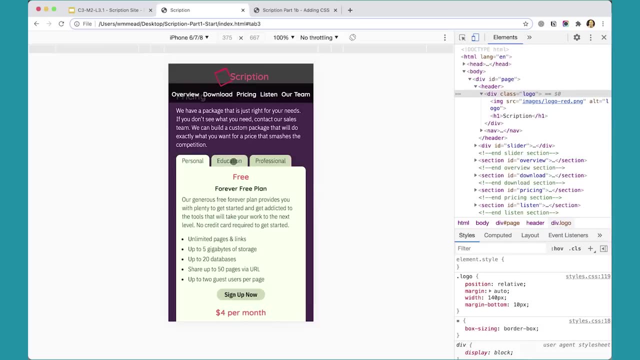 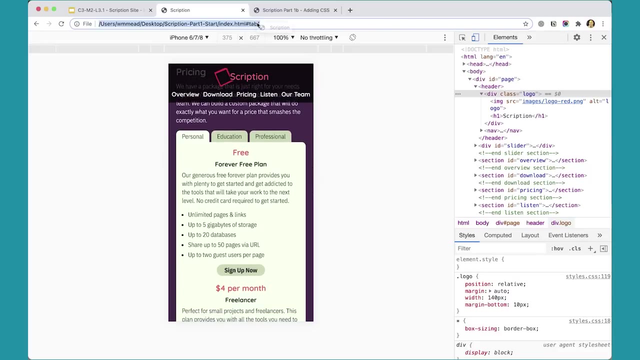 here and click refresh and just like magic, look at that. we have tabs, we have a tabbed interface. these tabs don't work because we haven't done anything with them yet and now we're, i'm getting those things up there in the header. i don't really want those there. 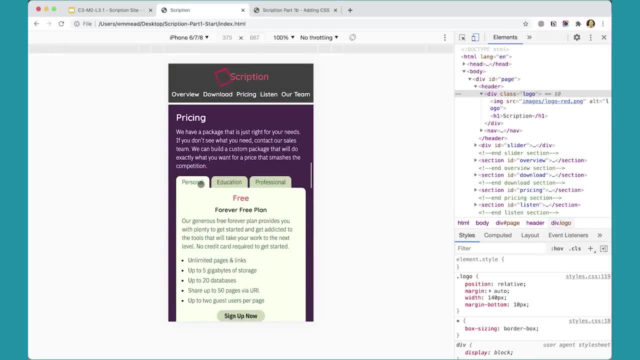 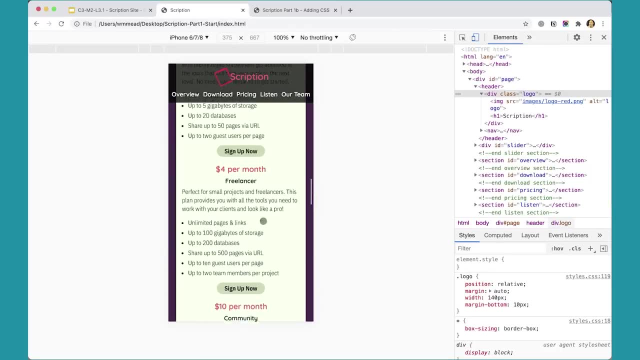 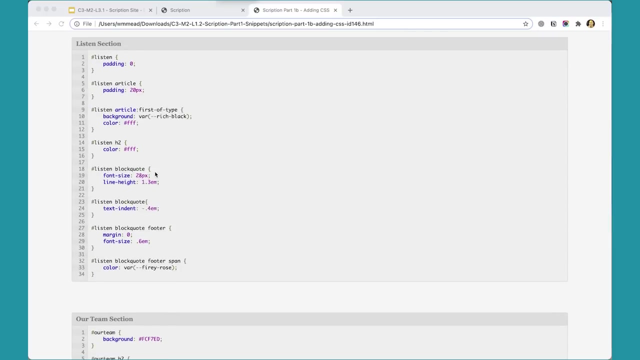 but, um, we'll get that to work later. that'll be great. let me get that to work, but we've got all of that content designed and looking pretty good. now we just need to go on to the next section. let's get the styles for the listen section, and it's not that many here, it's just a few. 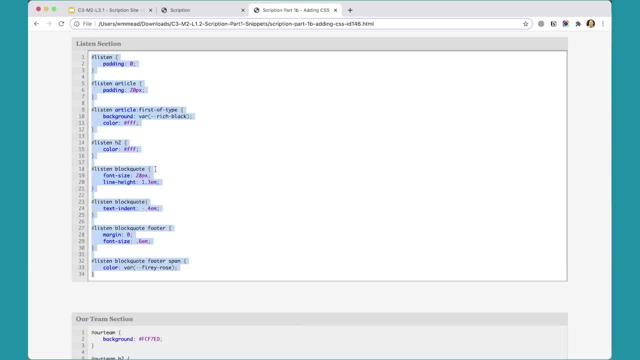 we'll add more. you'll add some more later when you do the job script to make the actual content rotator work. we'll add a few more, but we'll get those into place and then let's come back over here and put these in just to kind of get that to display properly. 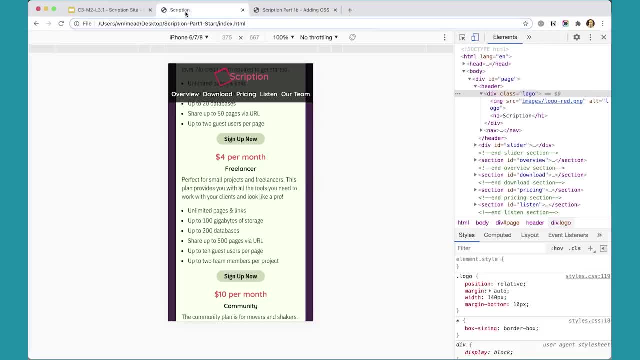 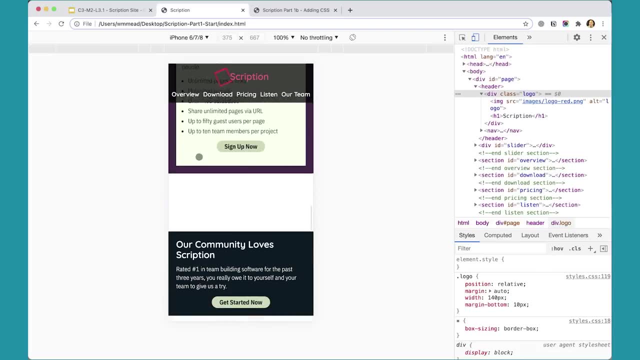 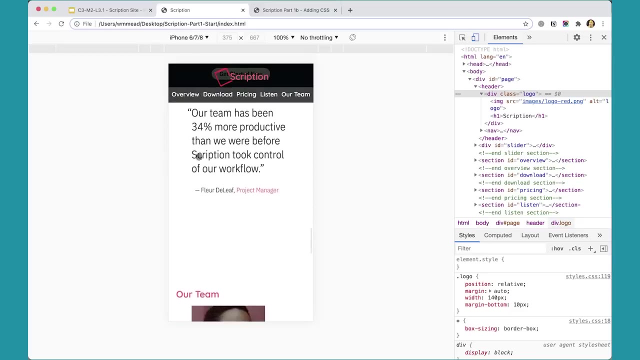 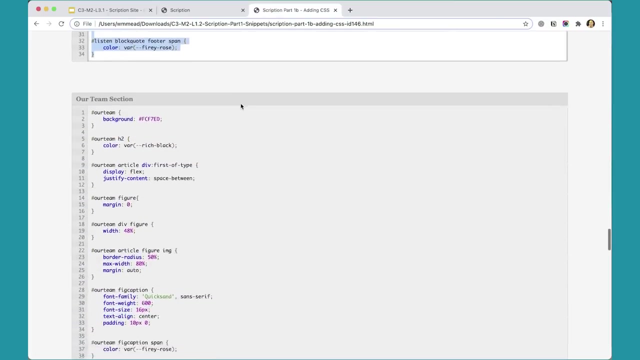 save that and then let's take a look and see how that is actually coming through. refresh this, scroll down and here's our listen section. looks nice for mobile. next we've got the our team section. let's go ahead and add that there isn't going to be any interactive elements for the rest of the page, so 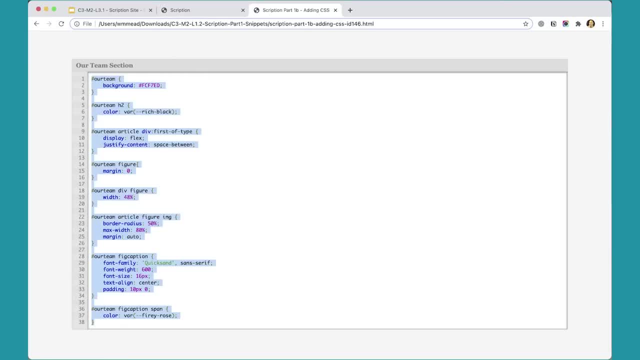 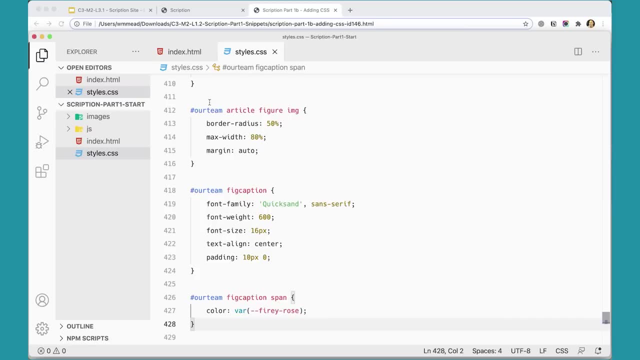 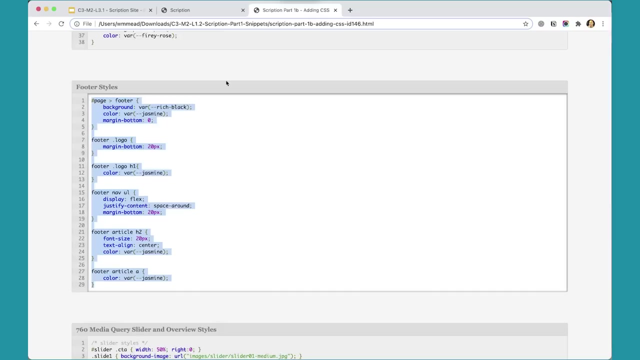 these styles will just stay the way they are and we're not going to do anything interactive with these. these last two sections, the art group in particular, but let's just go ahead and do that. so the rteam part and the footer. And again, if you're not sure what these rules are doing, 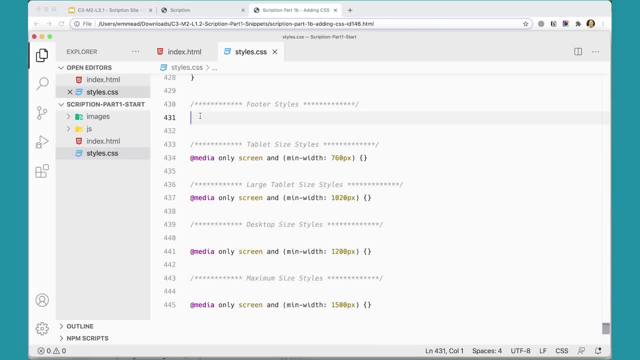 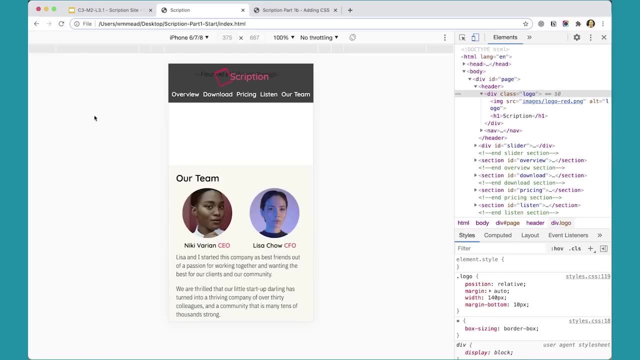 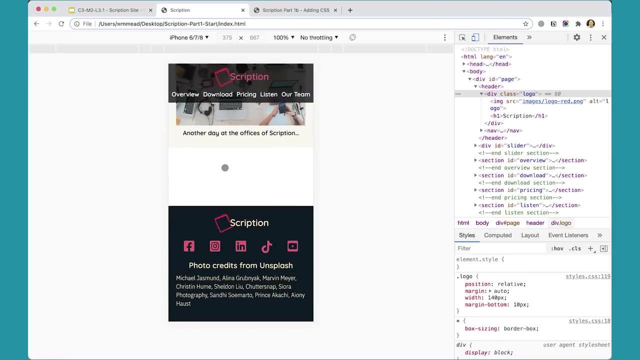 we recommend playing around with them. Take some time with it to see what they actually do. Save that. Let's come back and see how the rest of our page shapes up. There's the rteam section for mobile and the footer, And now we've got the entire mobile version. 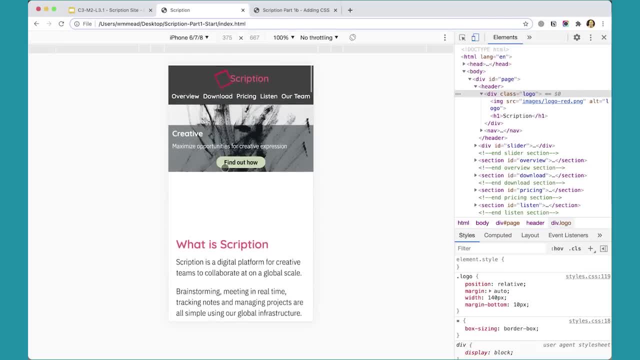 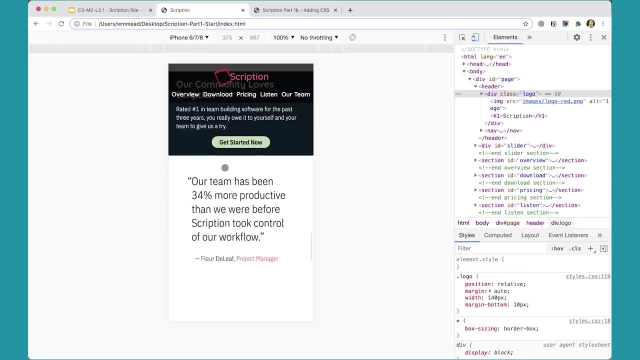 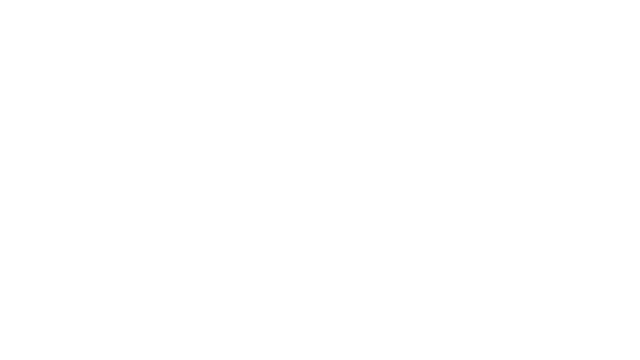 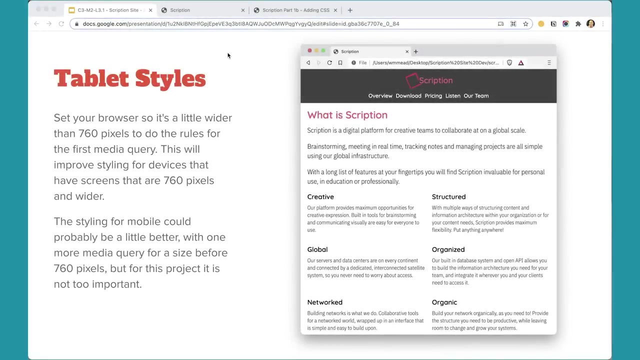 of this page set. The next thing we need to do is add- well, adjust- styling in the media queries for when the page gets larger. So we'll do that next. You've finished the styling for the mobile version and now it's time. 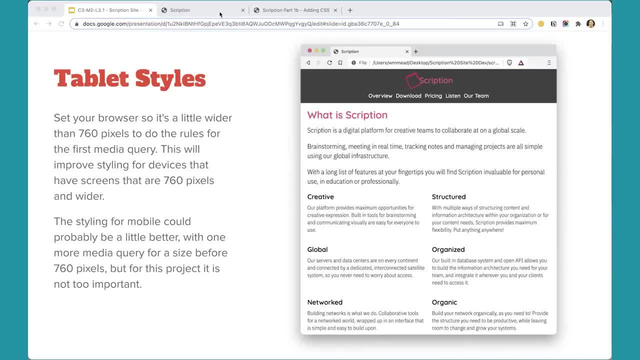 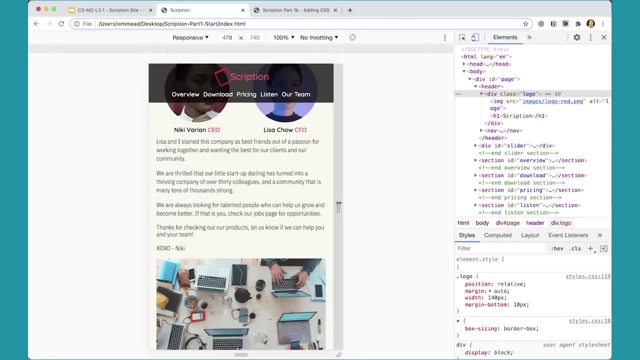 to get the styling in place for the tablet version. So to get ready for that, come over here to your view, switch this to responsive and make the screen just a little bit larger than 670 pixels. What did I say over here? 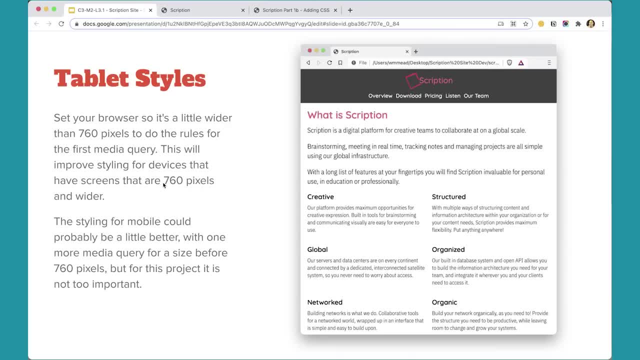 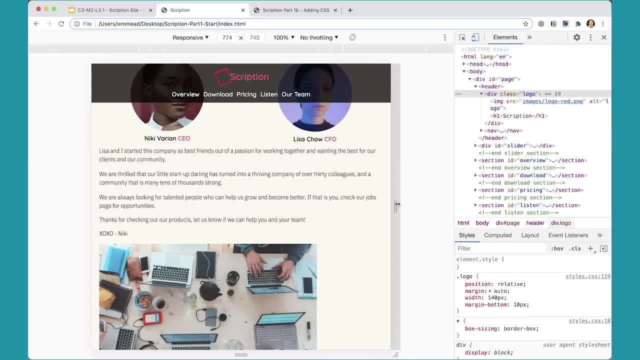 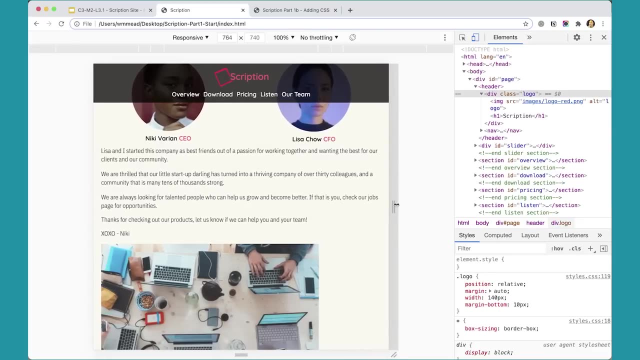 I've forgotten now 760.. 760 pixels And honestly I probably could do a little bit more. but you know, I'm not sure if I'm going to do more for the styling in between these sizes, but somewhere in here, 761.. 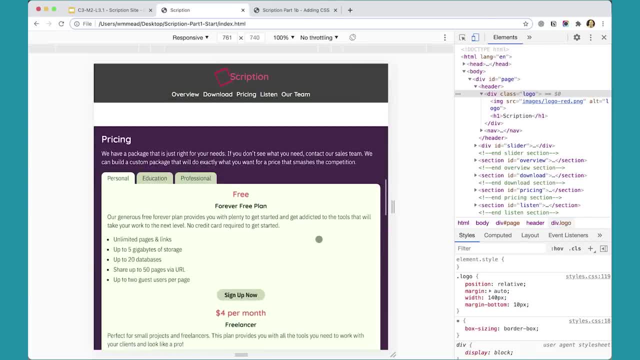 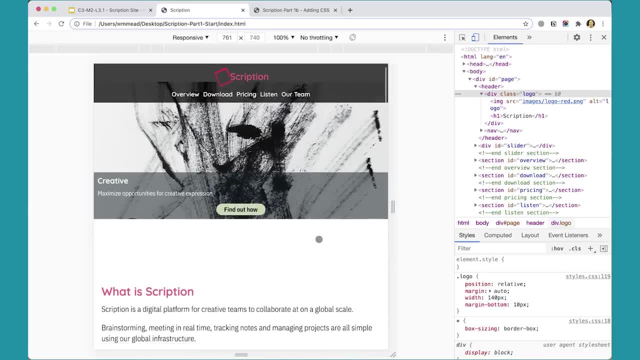 Sure, that's fine, But at this point we're getting to a point where our layout just doesn't look quite as good. at this size We could do a better job, And so we can add a media query and kind of adjust our layout a little bit. 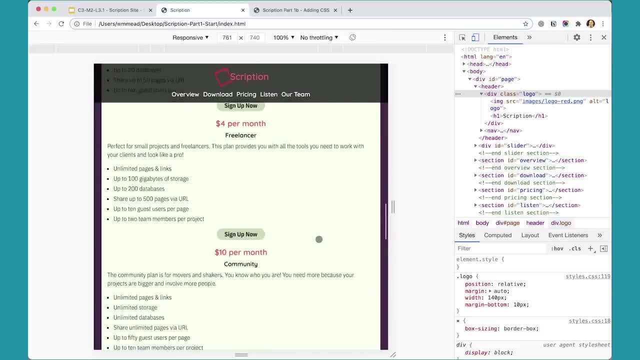 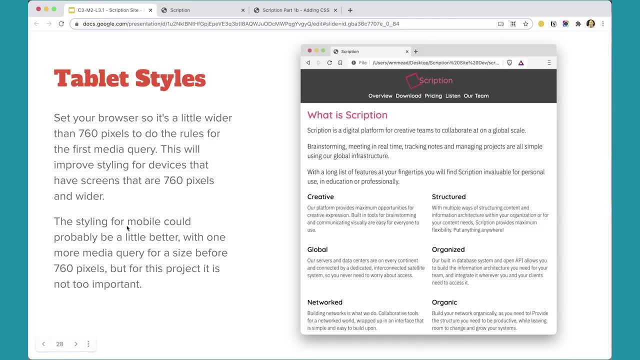 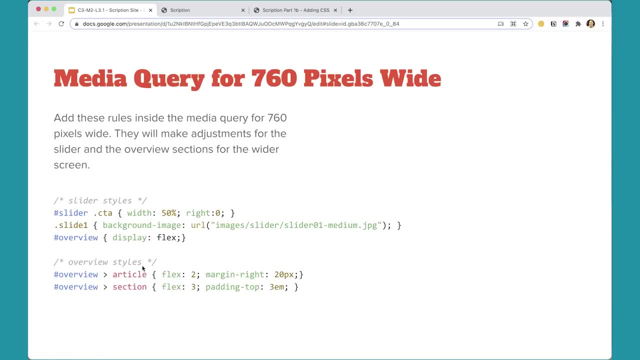 based on this size. here And again, we'll just copy and paste our styles in place So you can kind of get a sense of how that could work. Okay, So once you've got that set up, let's go in and add some styles for our media query. 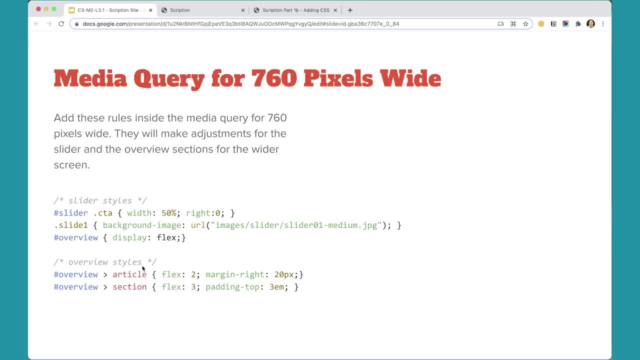 And again, Visual Studio Code's going to mess up my formatting for these, but that's okay. I kind of like them when I'm putting stuff inside the media query. I kind of like things to line up all in one long line. 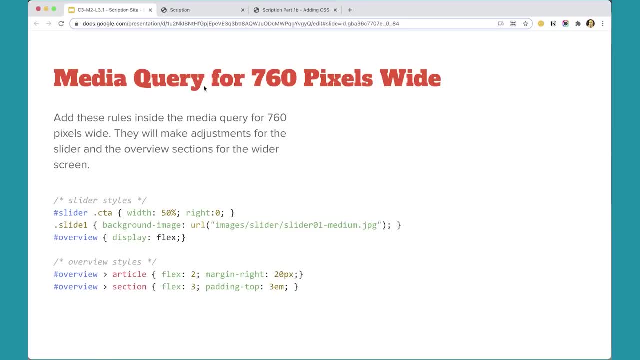 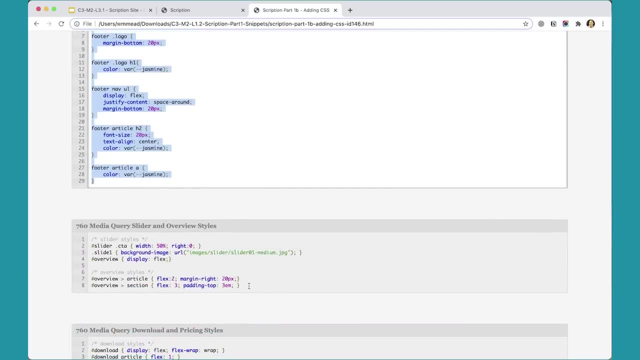 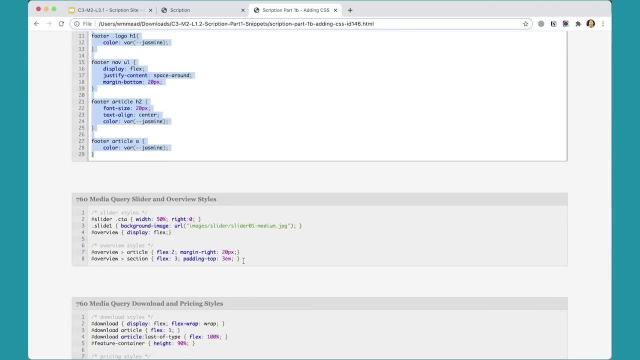 rather than to sort of expand out. But Visual Studio Code's not going to cooperate with me on that, but that's okay. So I'm going to add some media query 760. media query styling for the slider and for the overview, to kind of make those two areas. 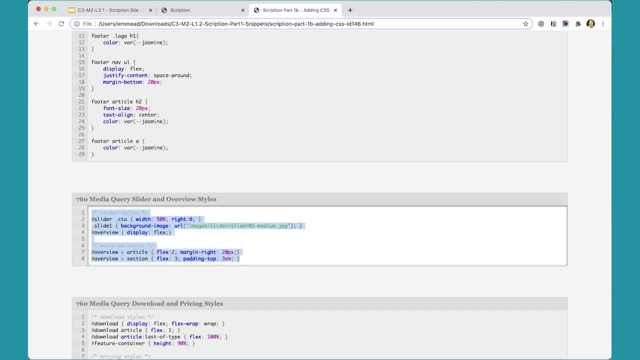 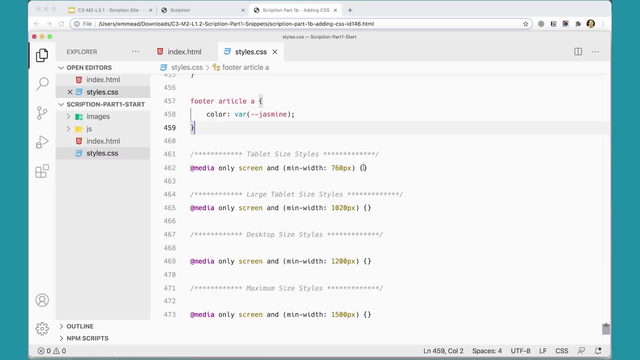 look a little bit better. So I'm going to copy that, come over here and scroll down And you can see I have a media query here for 760 pixels. So these rules are going to be set up. I'm going to go between these two curly braces in here. 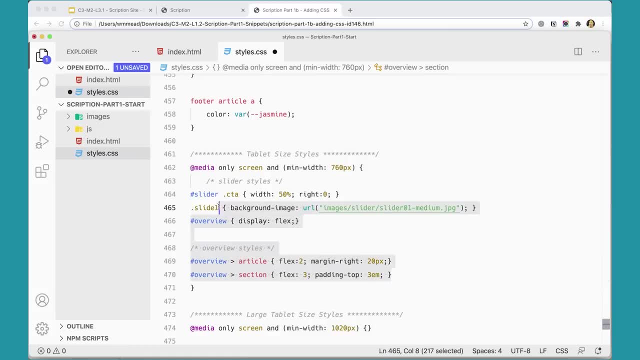 I'm going to paste those in and even tab them in a little bit there. When I click save it's going to expand them all, which kind of drives me nuts. but that's all right. But if I come back and look at that, 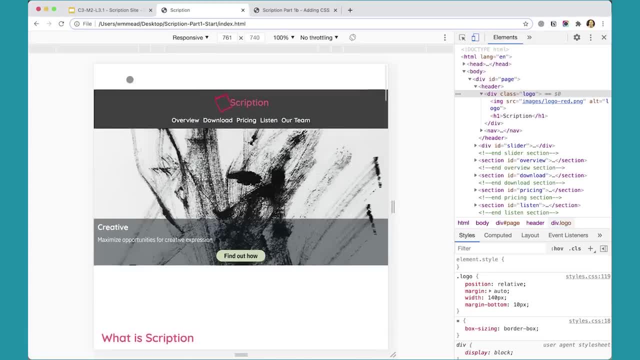 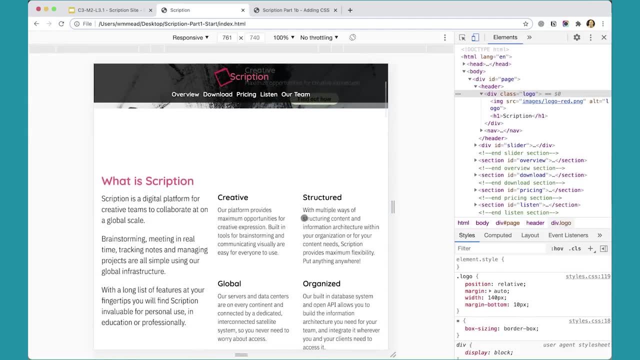 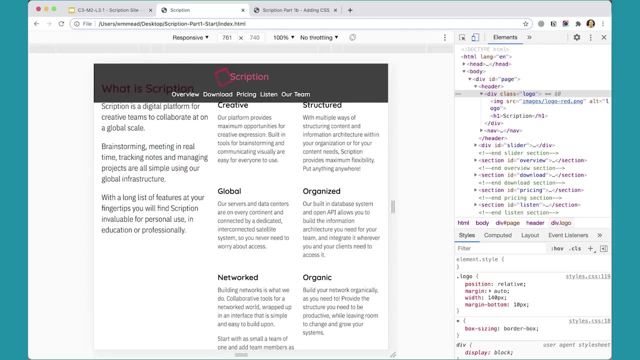 if I come back here and refresh up at the top of my page, you'll see it's adjusted this down here. it's made some adjustments to this area And basically what I'm doing here is I'm just overriding some of the styles that are up above. 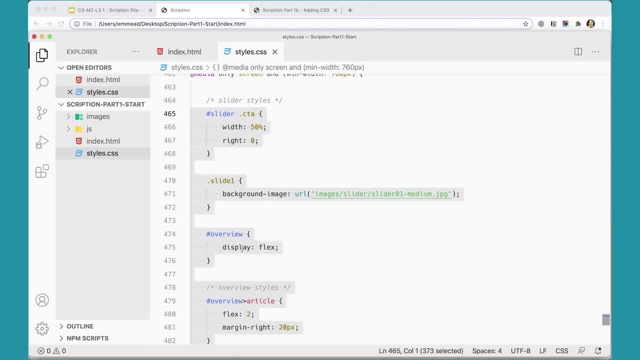 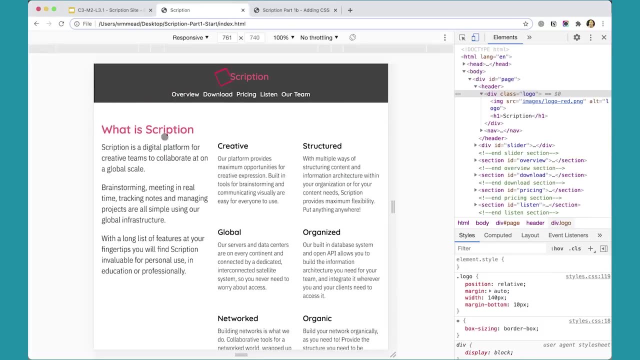 with some slightly new versions, set overview to display flex, for example, so that I can get this entire section here, So I can get this column sitting next to these columns rather than all just one column By the time I get to 760 pixels. 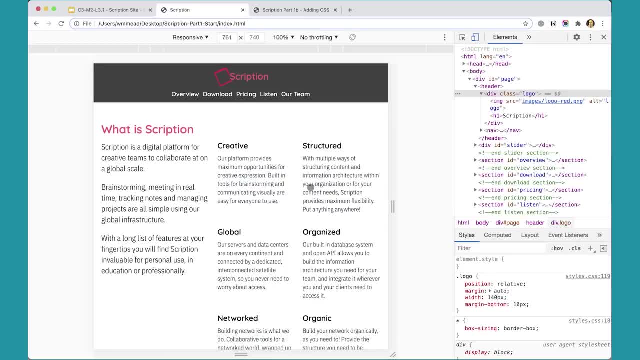 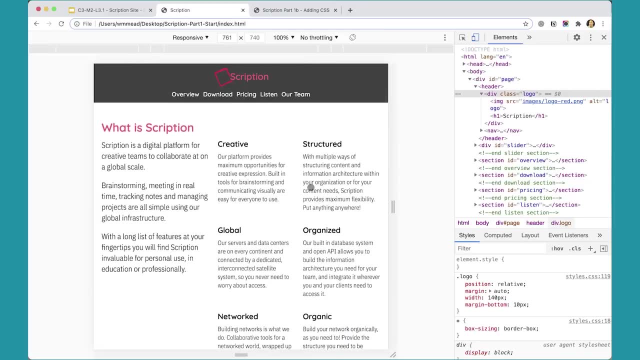 I've got enough room for some additional columns. So it's a lot easier to add layout as the screen gets wider than it is to take it away as the screen gets smaller. So that's why we start with mobile first is that we can easily just add layout. 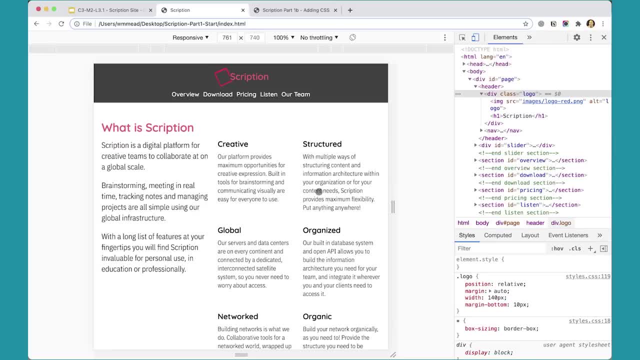 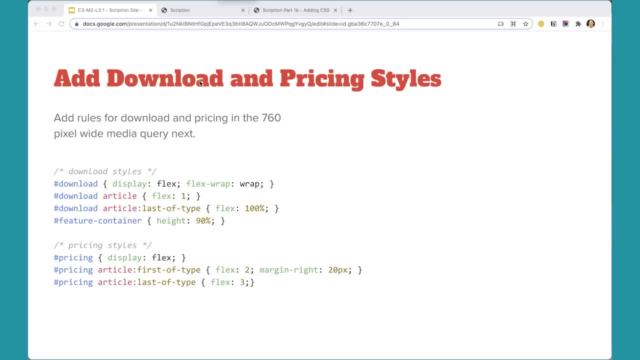 by just telling the section to display flex and just add a few rules to add some layout as the screen gets wider. Okay, great, So we got that into place. I have a few more rules for the download and pricing style sections. So again, they're just giving me some layout. 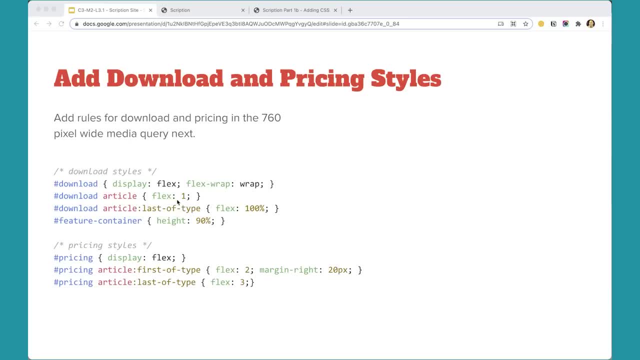 by saying display flex and flex wrap, setting the article to flex one, just giving me some layout, since I've got enough screen space to do it here, And all of these are actually just providing a little bit of layout using the flex box model here. 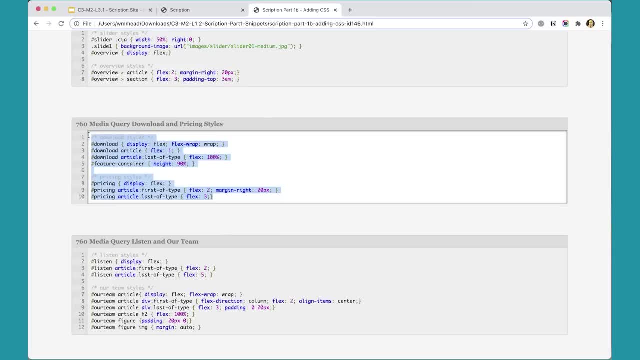 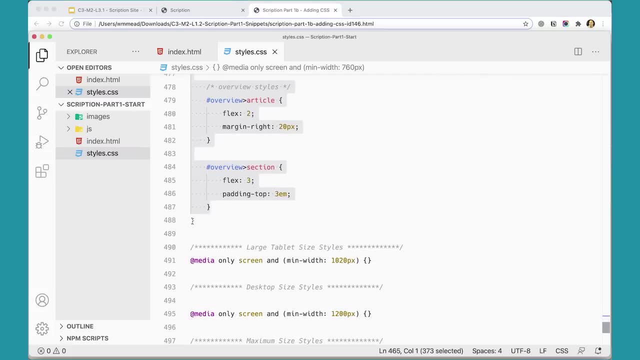 Flex box layout model. And again, these are gonna go into the 760 media query. So just after these rules here, but this is the closing of the media query here. that curly brace, Don't lose that, So that'll screw things up. 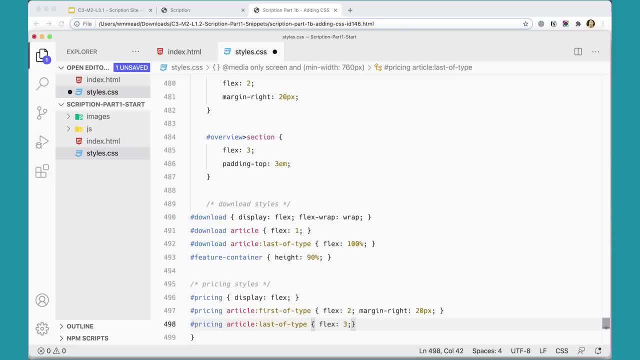 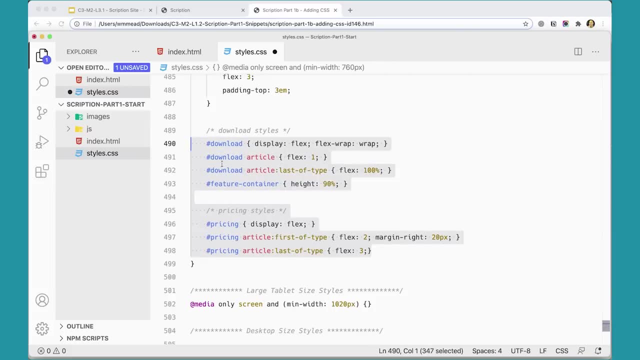 It goes after that one, And I wish that it didn't do this thing where it piles them all up. In fact, I'm gonna leave those like that and not save it until I go and get them. I'll get the next set. 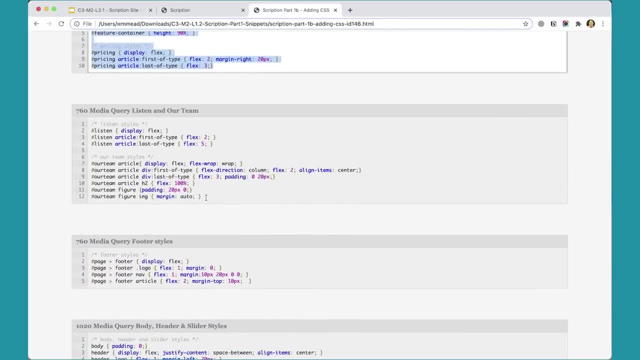 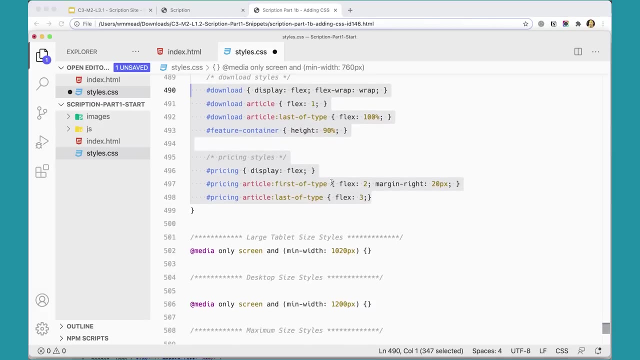 which is for the listen and our team, And then we'll do a few minor changes for the footer as well. So let's go ahead and put all of these in And again, if you're not sure what these do, I recommend 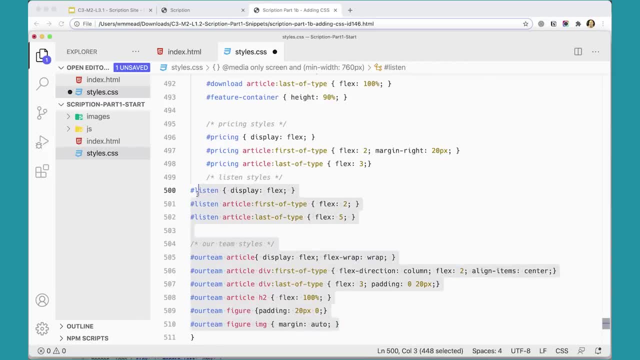 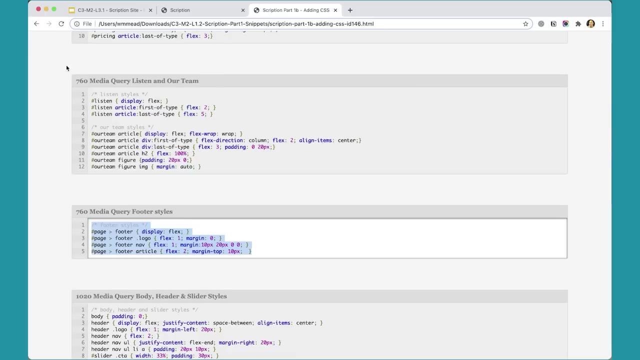 I really recommend coming in and messing around with them, Seeing what they do, Take them out, See what happens. We've got that, And then we've got the ones for the footer as well, Hopefully, and I realized that by copying and pasting this stuff in. 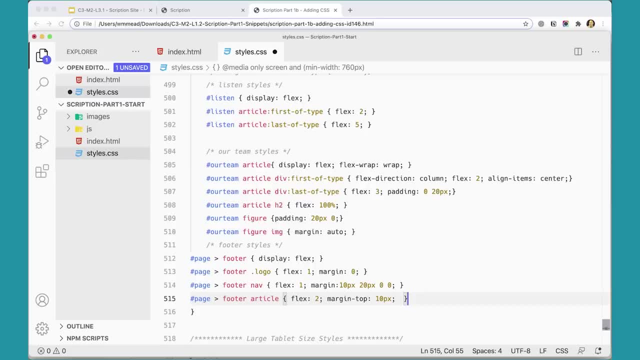 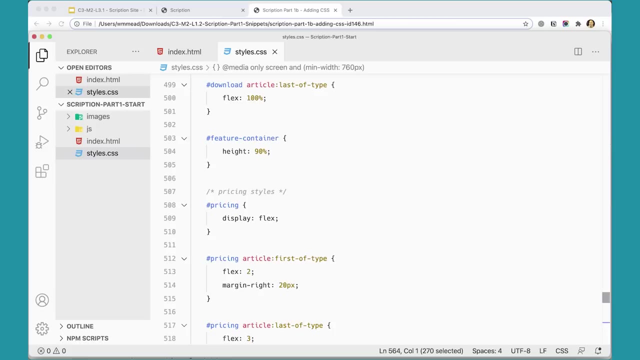 you're probably like: well, I'm just copying and pasting without really understanding and sort of following along. But hopefully some of this sort of sinks in a little bit in terms of seeing the page come together so that when you start doing the interaction design stuff it'll make more sense. 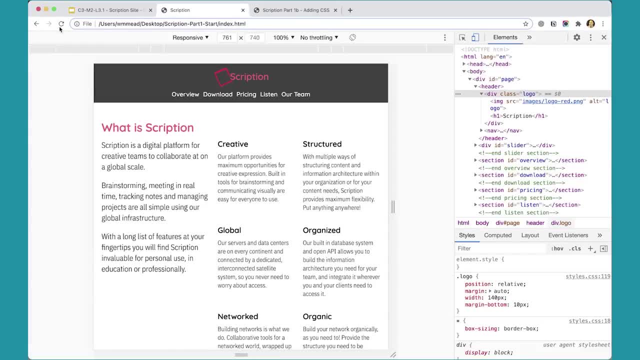 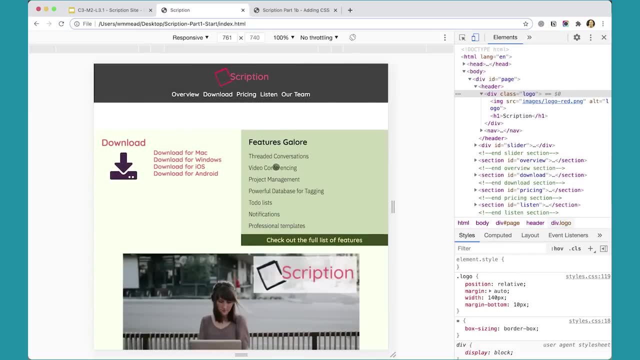 That's my hope, But if it doesn't feel like it seems like it's doing that, then that's fine. You could skip to the end. I will provide this file for you finished, when we're done. You can see I've added a little bit of layout here. 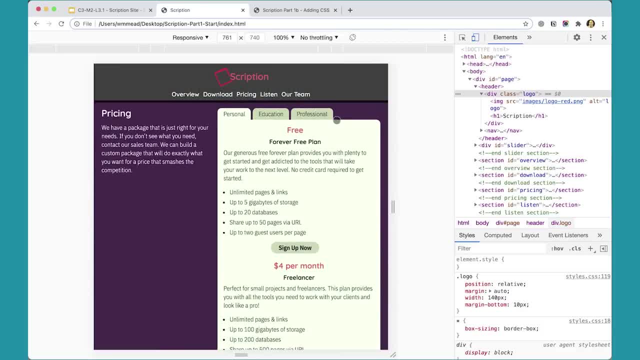 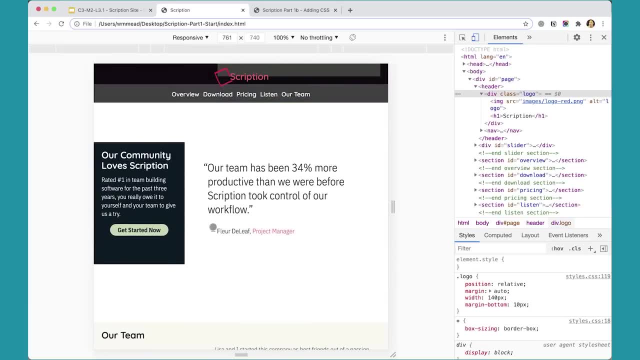 Down here. I've added a little bit of layout. now. Pricing is over here and my tabs are on this side instead of one on top of the other. This is now on the left instead of on the right, And then I've added a little bit of layout on top. 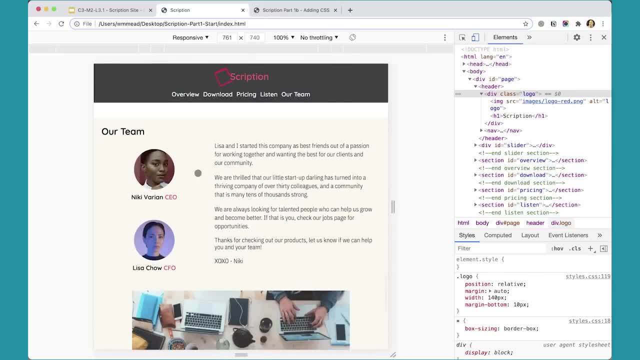 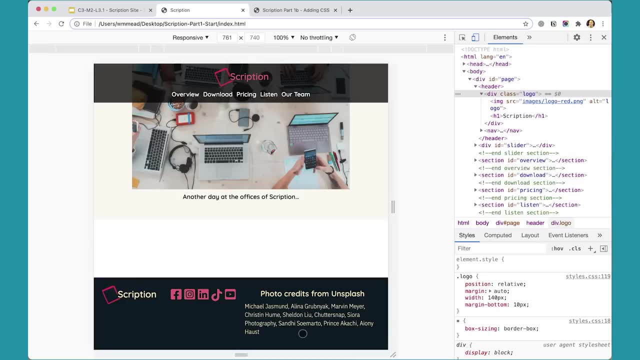 And then we've got our quote here, which we'll use. our content rotator for The R team has been reconfigured to make that look a little bit better. And then the footer is set up to look a little bit better, By the way, in the footer. 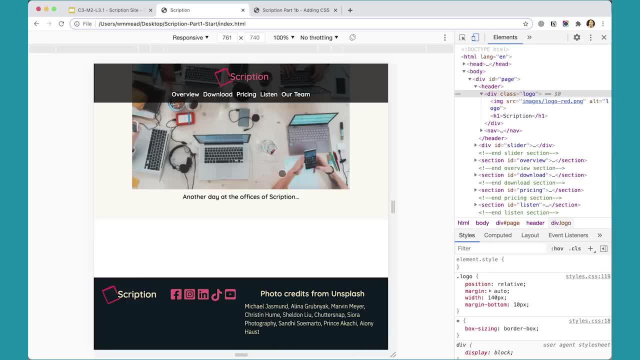 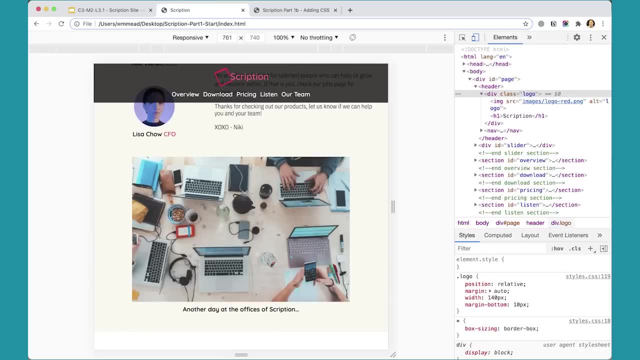 I have the names of all the different people who provided these images which I got off of Unsplash. Okay, great, We've got the 760 media query done. Go ahead next and work on the next media query for the full desktop size. 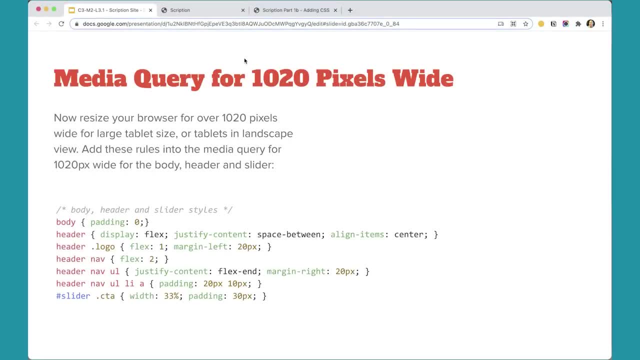 The next break point for my media queries is 10, 20 pixels. When I get my screen that wide, I want to make further adjustments to the layout And we're really getting much closer to the design that you saw over here on my Adobe X. 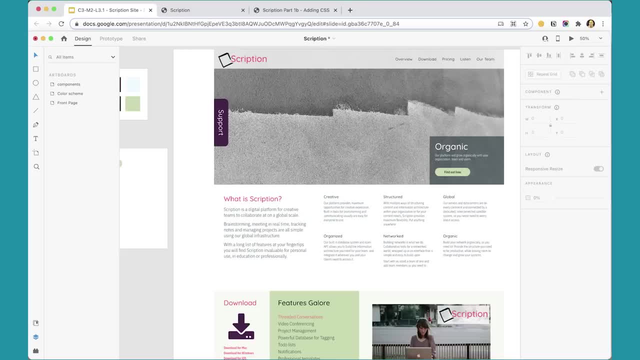 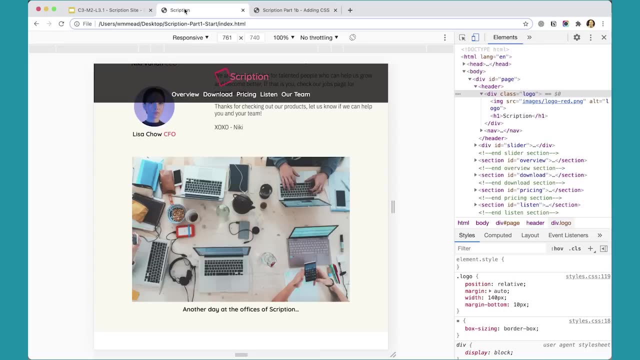 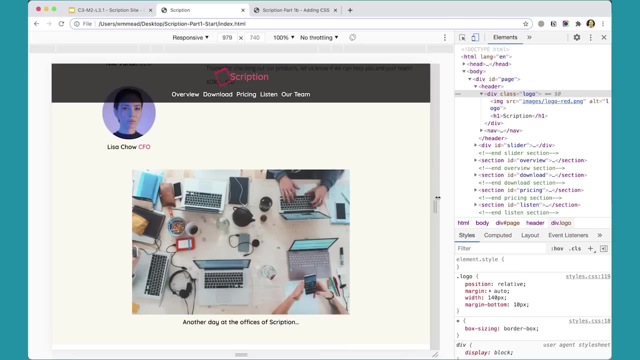 The file. at that point we're leveling more, but we're getting a lot closer to that. So come over to your thing here and set this so that it's 10, 20 pixels wide or a little bit wider, And I might need to move this thing down. 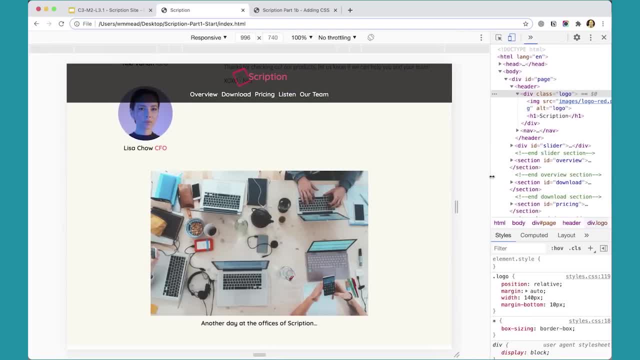 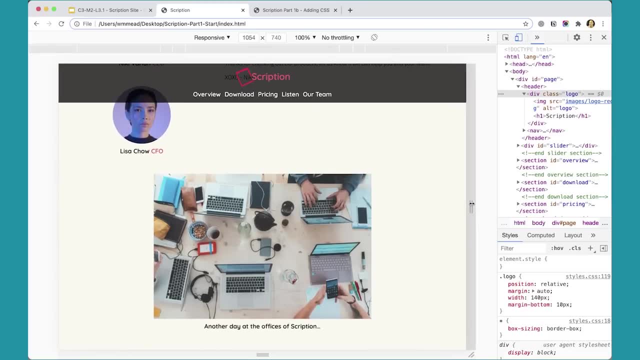 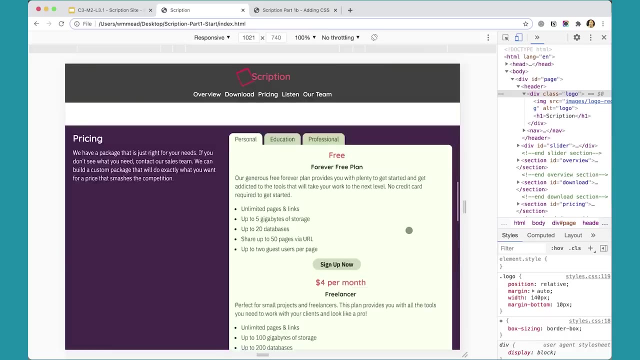 or maybe make this a little bit smaller here: 10, 20,, 10, 21,. that's plenty. There we go At this point. if you look at this, the visual relationships just aren't as good as they could be. 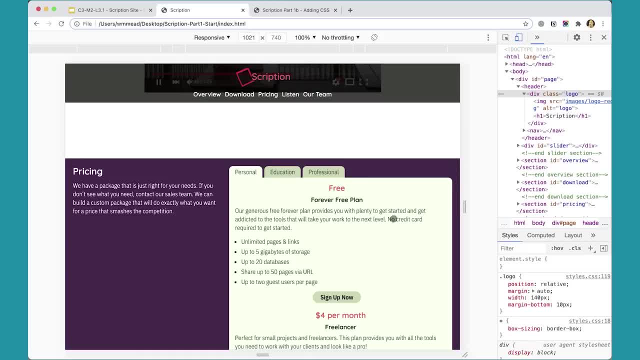 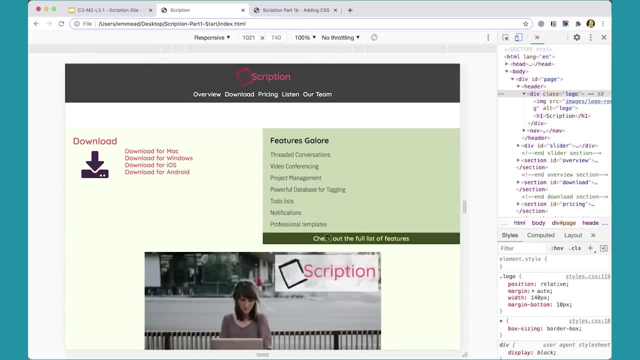 Like this is too wide in here. I've got too much space in here. This is kind of squenched in here now, So this is where I want to make some adjustments. Here too, this looks kind of funny Like maybe if narrow enough. 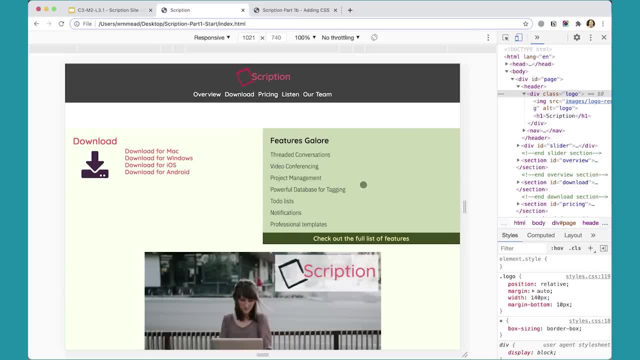 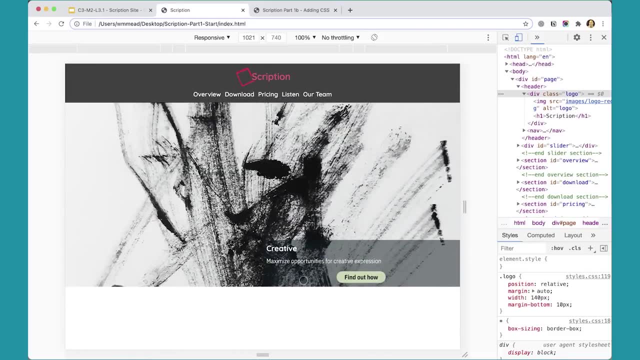 wide enough now that I can get all these three things kind of in a row here. So we just want to make some adjustments to how these different elements lay out and the space available for them to make them look a little bit better. And this is all just part of what you do as a designer. 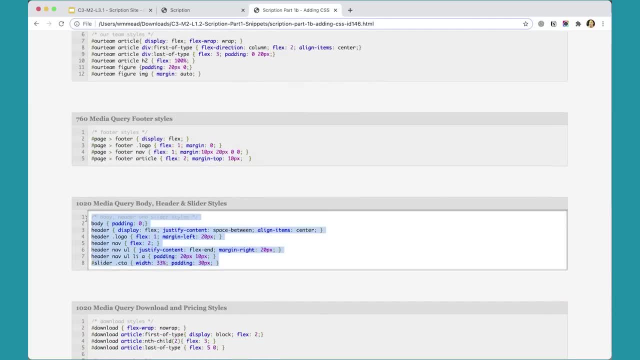 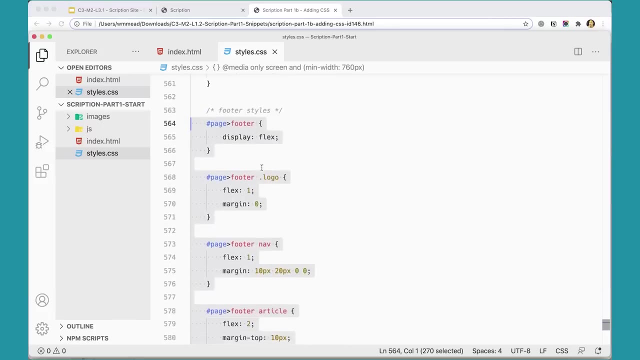 So I'm going to come in here, I'm going to grab these rules here for the body, the header and the slider styles. Just got some basic styling changes that I want to make happen here And we will put those inside of the large tablet size. 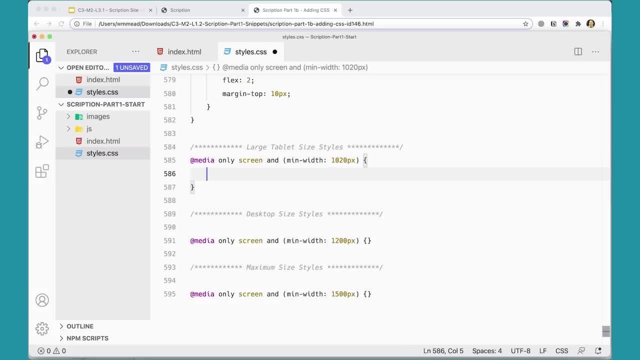 10, 20 pixels. stick them in there. That's going to take care of those elements. The body, the header and the slider all get slightly different layout, different, slightly different padding. You can tell all this stuff has to do pretty much. 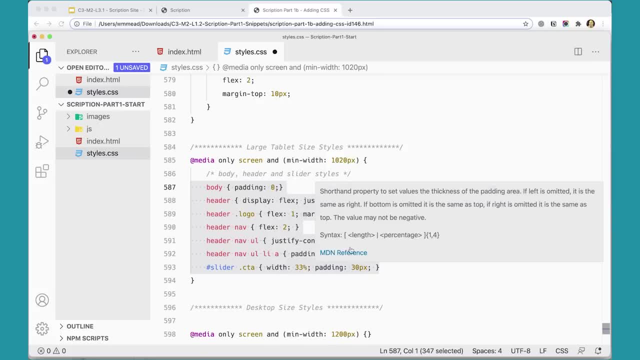 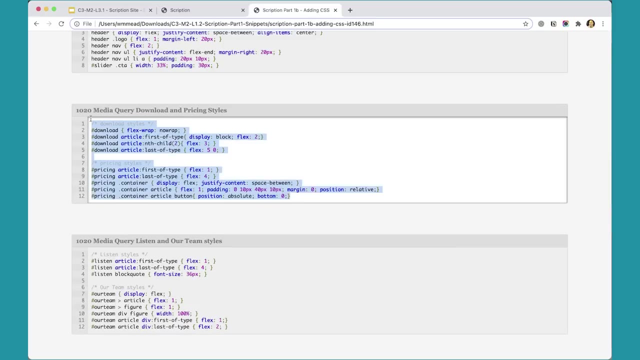 with the layout with 33% adding 30,. you know it's all having things to do with layout in here that I'm applying to these elements And again, if you want to mess around with it, feel free. We'll add these ones for the pricing. 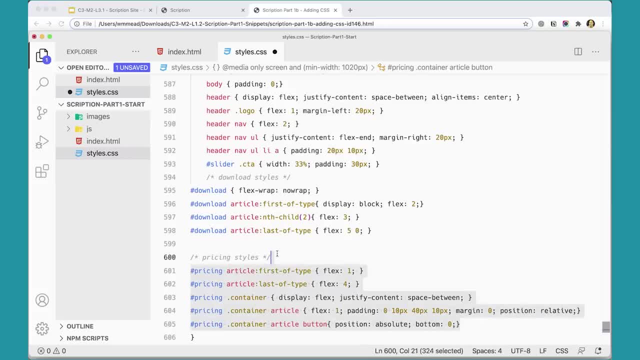 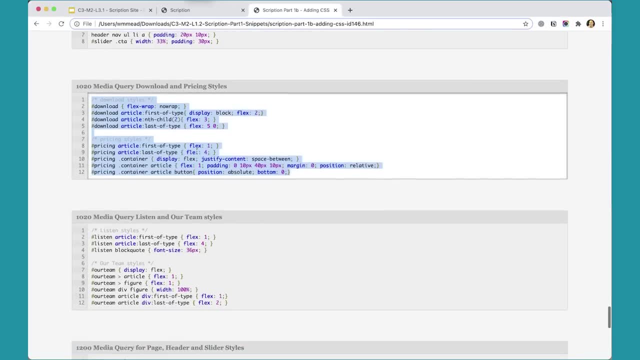 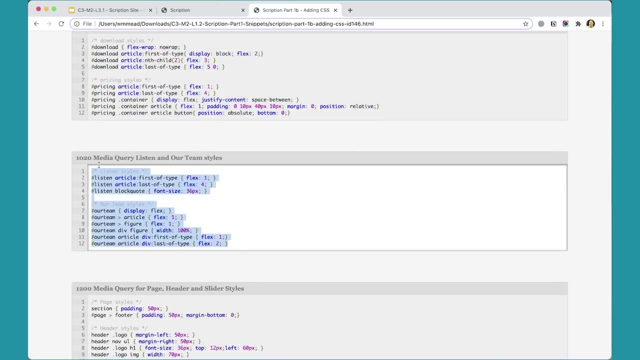 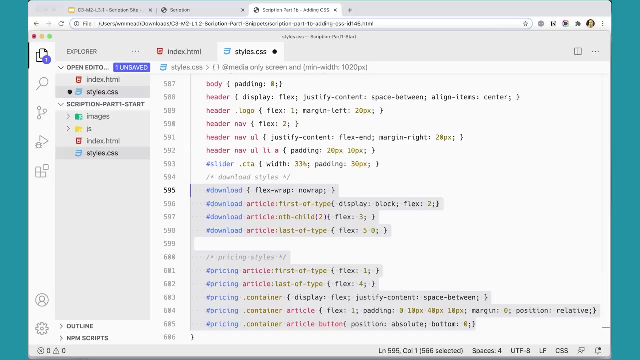 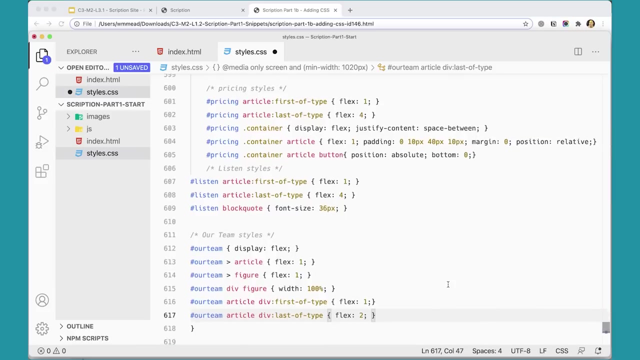 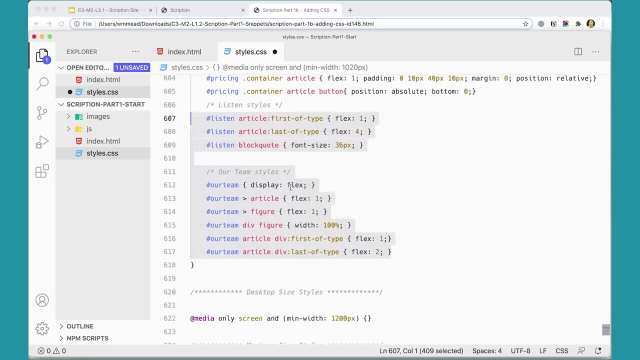 I'm going to add. that's the pricing and the downloads. This one is the listen and teams. You don't need to do anything for the footer, It'll just get wider Listen styles to have those in. you know, when I save, this is all going to get expanded, sadly. 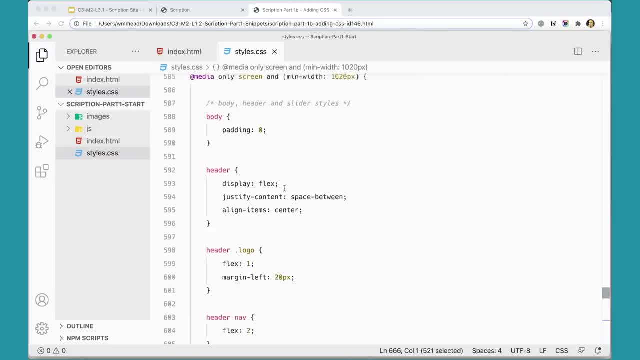 but there we go. Maybe you like reading it that way. The media queries: I like them all in one line. I find it. there's usually just one or two declarations, not that much going on. This one had more, but I prefer to put them on one line. 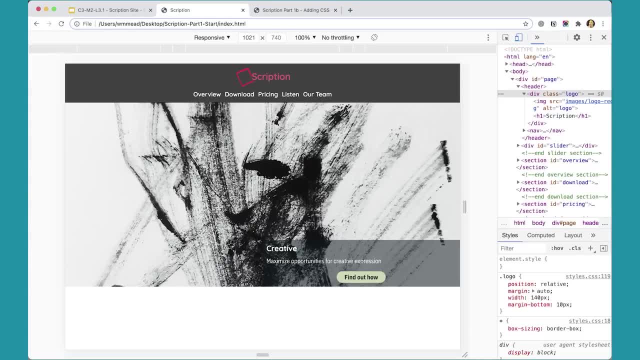 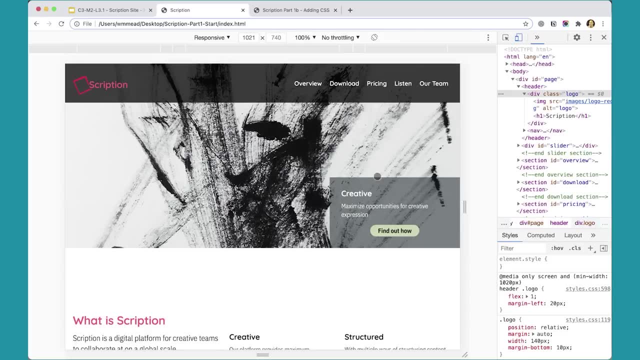 Let's go take a look and see what all of that did. So I'm going to do that. I'm going to do that with the navigation. There you go. So that's what I'm going to do for our 10- 20 version of our page. 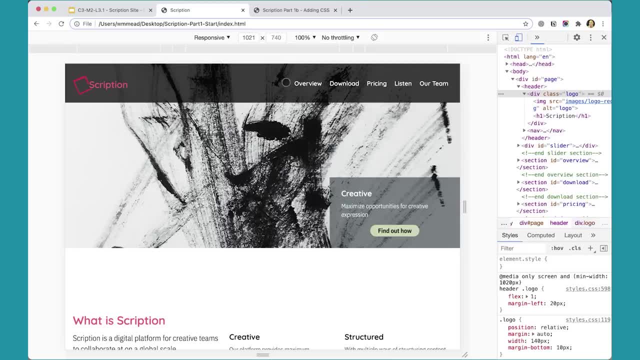 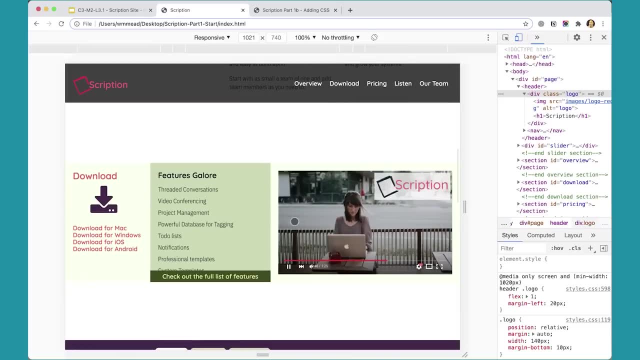 Refresh Now. this is now taking up a third of the width of the page. My logos over here, my navigations lined up down here. the spacing looks nicer for this Down here. this is all in one line, like I was mentioning before. 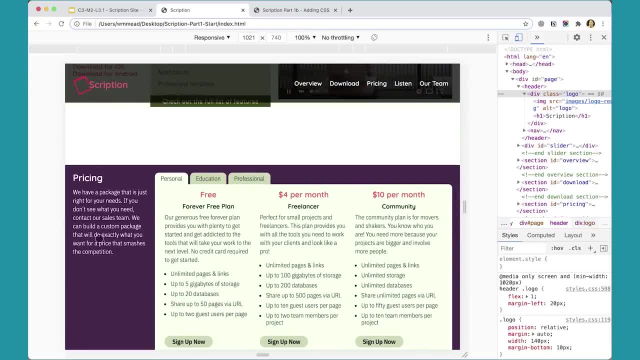 That makes sense. This is all set and ready to be animated, which is kind of cool. Over here, we've got less space for this thing and more space for the page, And I don't know why, but I think that's what's important here. 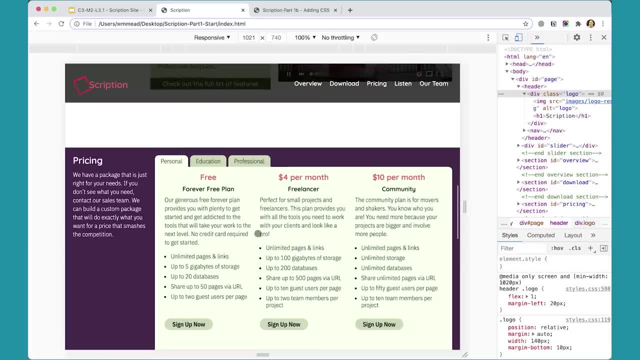 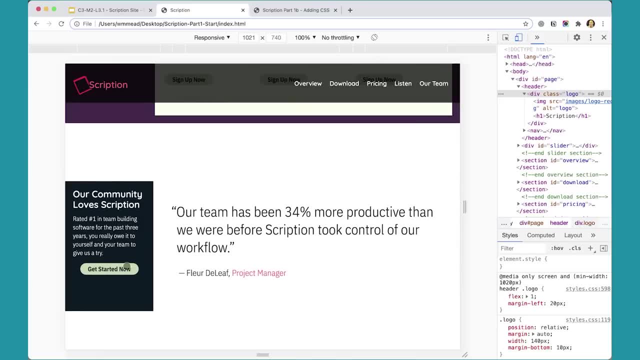 And I think it's because of the page size. more space for the tabs Makes sense. now that we've got more room for that. It's just a matter of coming up with the right proportions. Down here, this has been made smaller and this takes up more space. 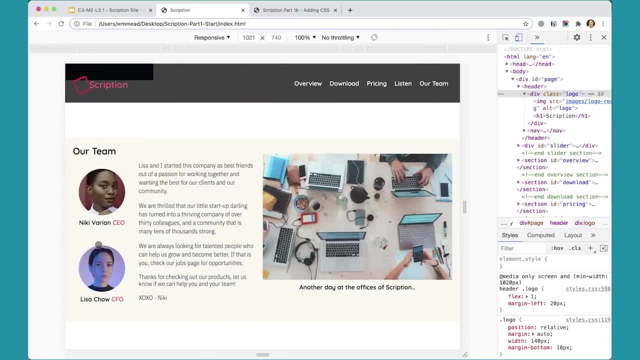 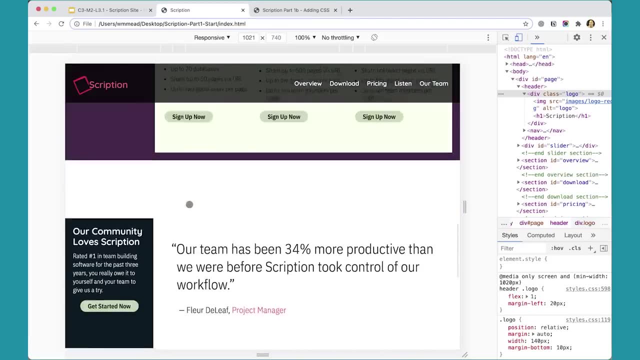 and the size of the font has been adjusted. This is looking slightly different with the picture over here now, so that's all in one row and the footer stays the same. There we go. The 1020 media query is done and our page is really coming together. 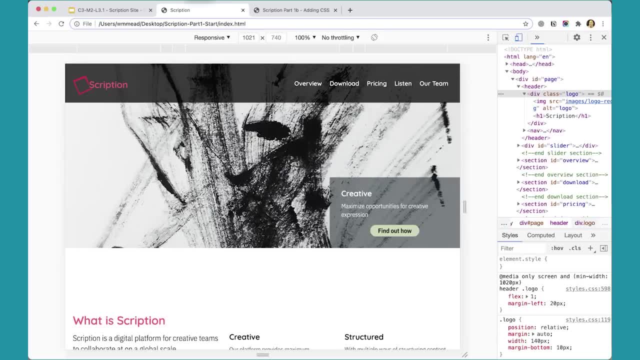 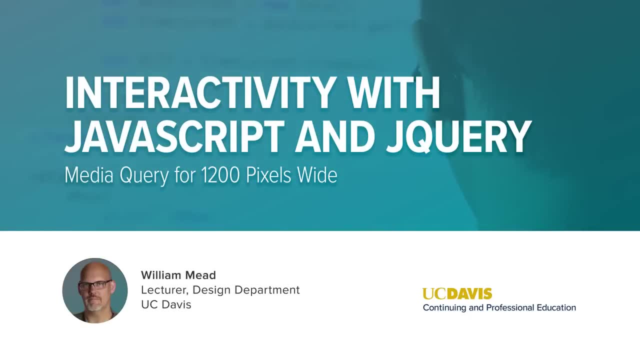 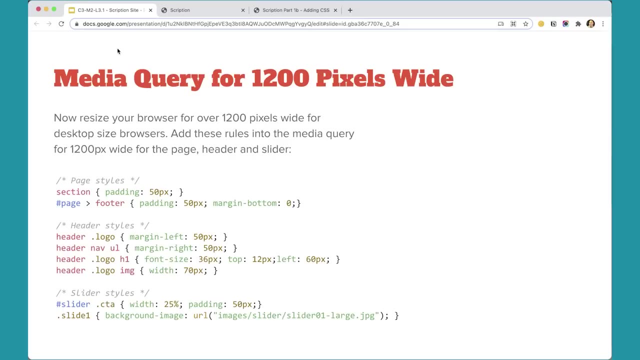 I'm gonna look at the next one in the next video. The media query for 1200 pixels wide is for when somebody's viewing this website on a nice large desktop and their browser's nice and wide and they've got lots of screen real estate. 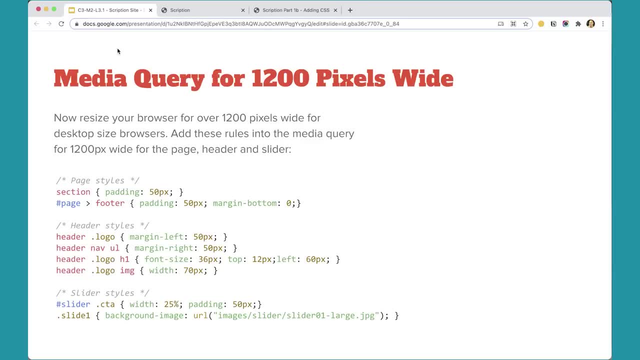 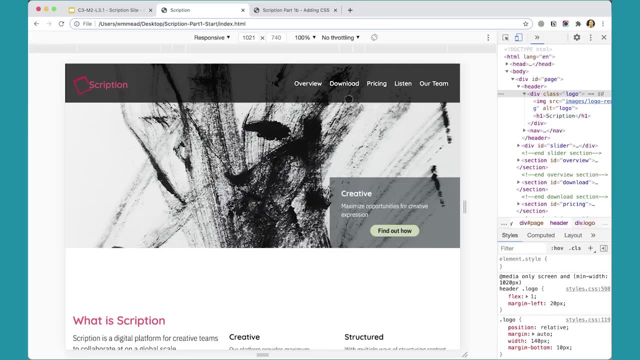 in which case we can really kind of optimize our layout for that look. So let's go ahead and add these rules in over there. You need to set your width here. For me to do it, I'm gonna need to move this thing down to the bottom here. 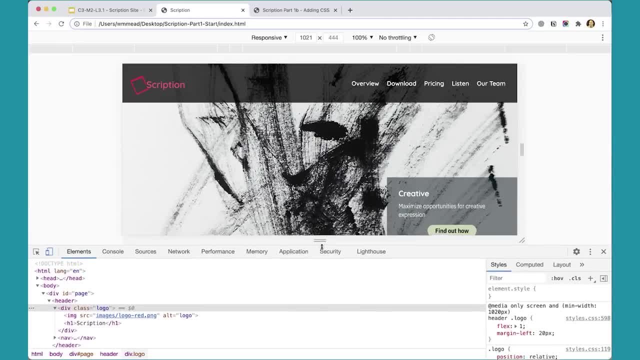 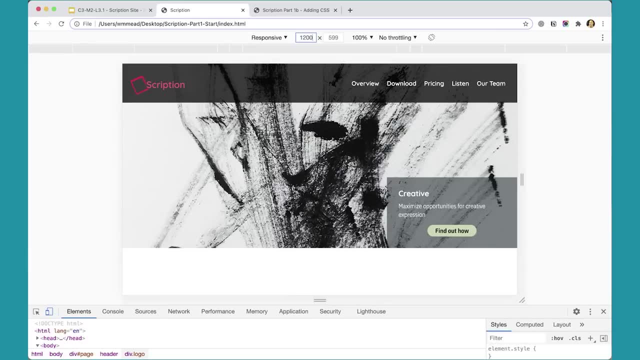 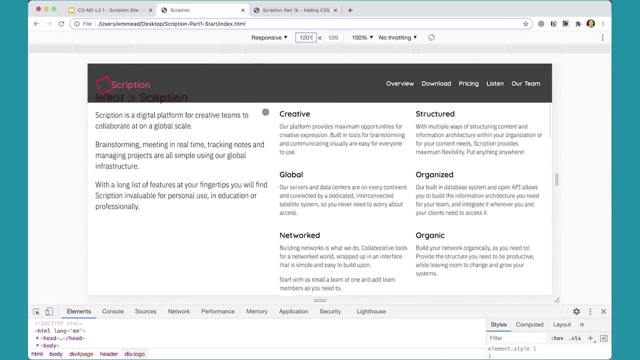 and I'm gonna shrink that down a little bit and then set this to 1200, maybe 1201, like that. Cause now I've got a lot, of, a lot of room so I can really do some nice stuff here. 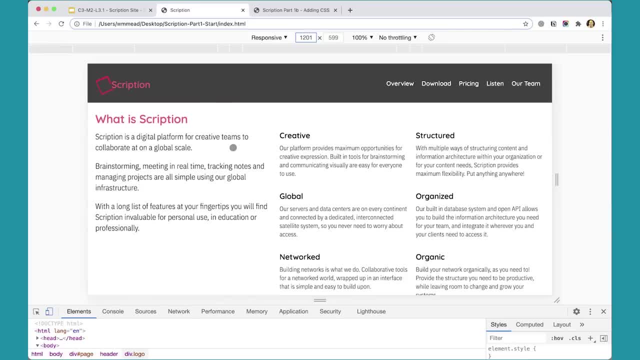 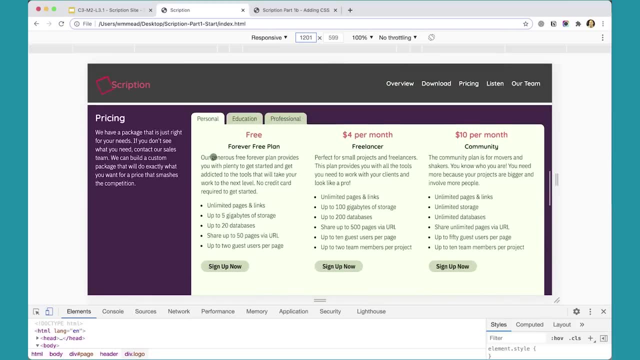 I'm gonna put these into two, into three columns instead of two. I'm gonna. this is too wide over here. I can shrink that one down, You know. just make minor changes in here. Some of them don't need much. 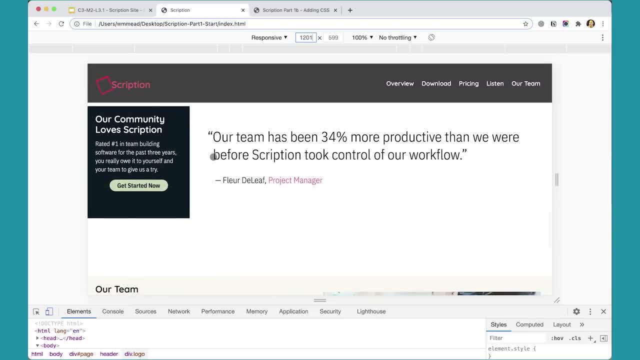 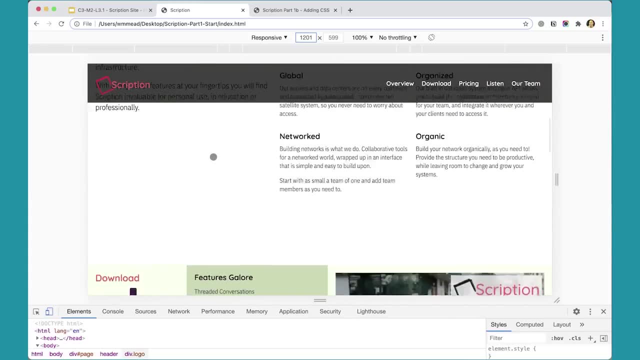 This one doesn't need a lot of change, but just making some minor changes to kind of make this stuff look a little bit better on the wider screen. So let's go over and add those rules that we have in our snippets, And they're here. 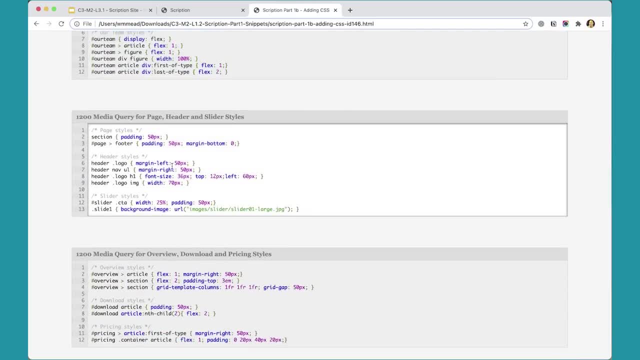 I'm gonna cut this, this set. first I'm giving you know sections, 50 pixels padding, So now I've got a lot of room. I can actually, you know, space things out, give them a little bit of room to breathe. 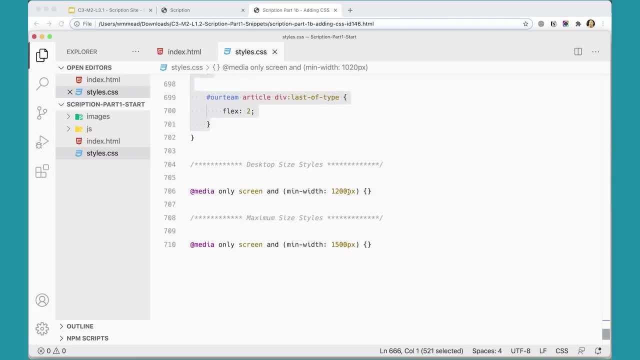 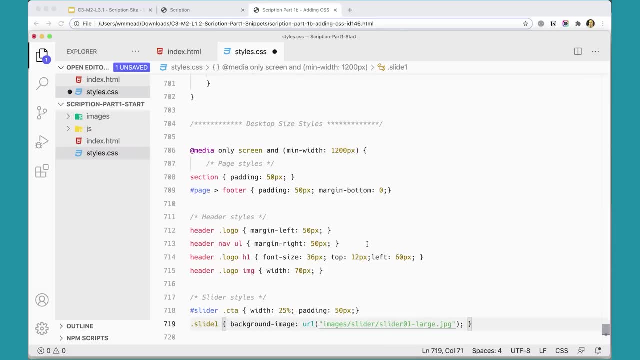 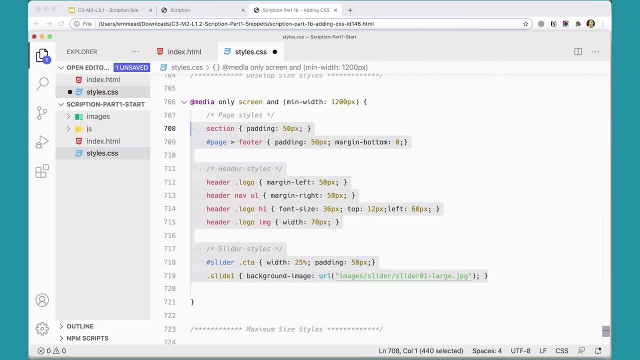 all of that kind of stuff. It all just has to do with providing some better spacing in here, And when you're a designer you wanna have. spacing is really important because it really helps communicate. So we wanna get that kind of stuff, just right. 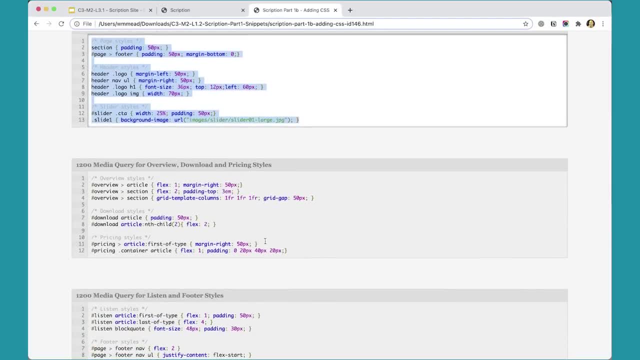 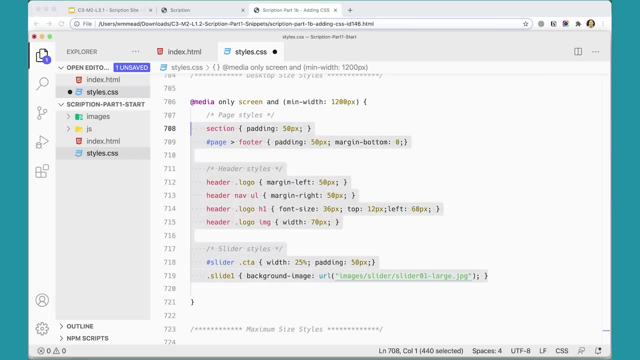 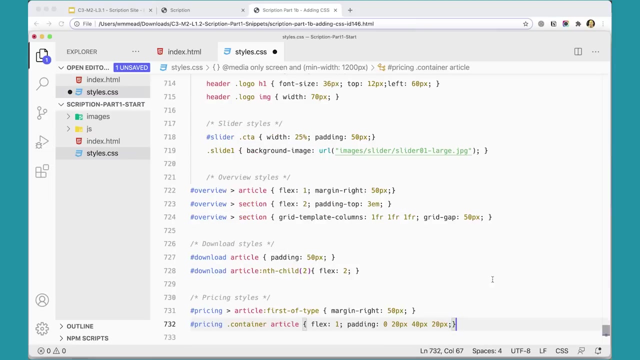 as much as possible. And then we've got a few more here for the overview: download and pricing styles: Oops, Switch to here and add those in Again. the angle brackets are there to make sure that only articles that are direct descendant of the overview section. 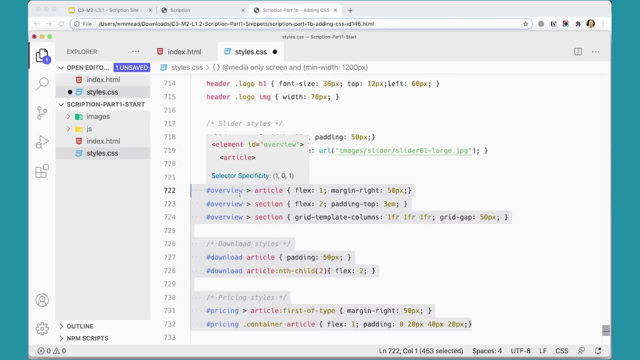 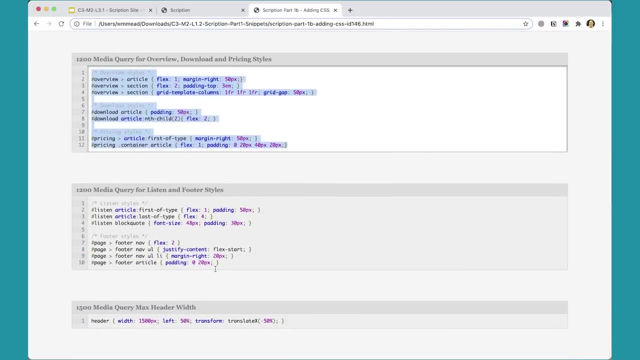 So it won't apply to articles inside, you know, an article inside of an article. It'll only apply to those parent level ones, And that's kind of helpful to be aware of. Okay, let's continue on here and get the last piece for this one. 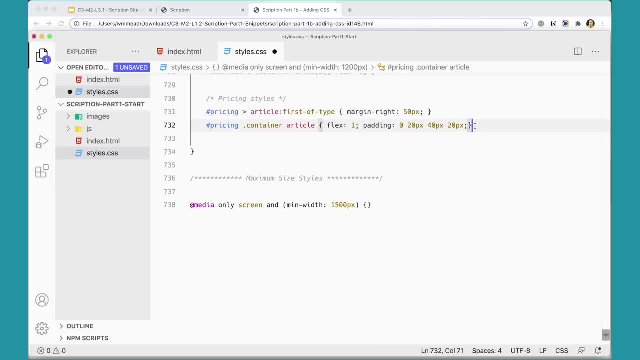 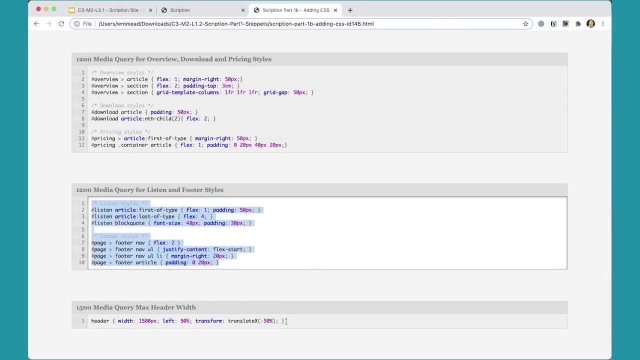 And finally put that in here. Footer gets some new styling at 1200 pixels to adjust for that. And then finally, we've got one little rule that goes in the 1500 or larger media query, And it has to do with the fact that the header 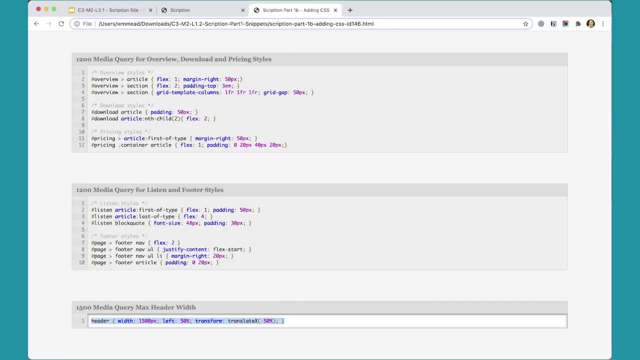 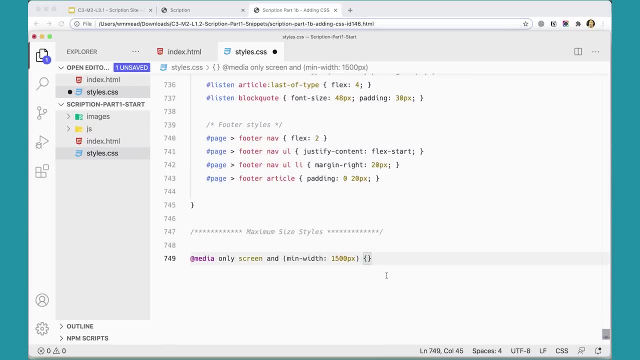 is set to fixed positioning, but I wanna make sure it gets centered in the screen if my screen is larger than 1500 pixels, which should be really large, And I can't even demonstrate that here in this video. but you'll have to trust me that it works, or try it out. 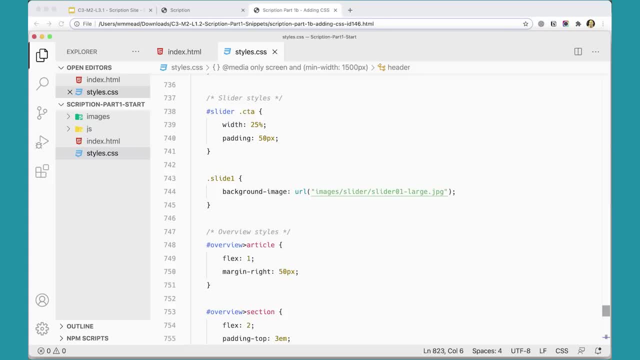 Or if you've got a nice big monitor, you'll see the difference. Take it out and see what it looks like without it and then put it back in. So now I've got that all sort of sorted out And in there I can come over and take a look at my page. 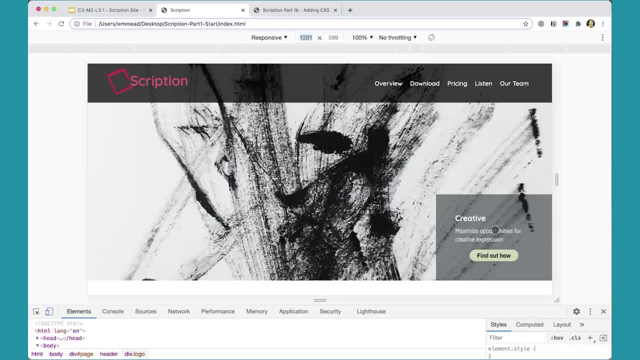 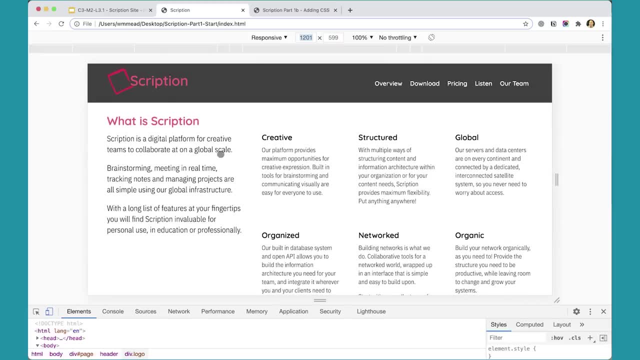 You can see this got reconfigured even smaller to fit a little bit better Down here. I've given 50 pixels padding on the edges, 50 pixels padding. I've got some. I've got some room here. It's nice to have some room. 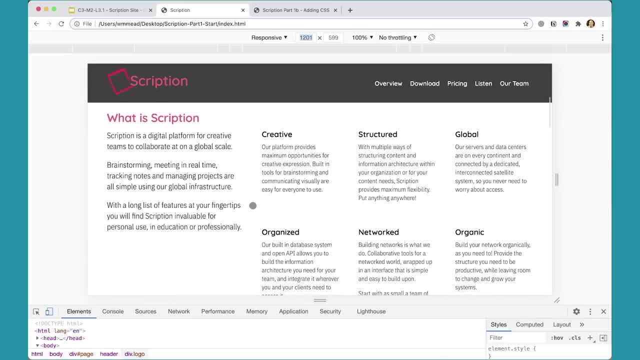 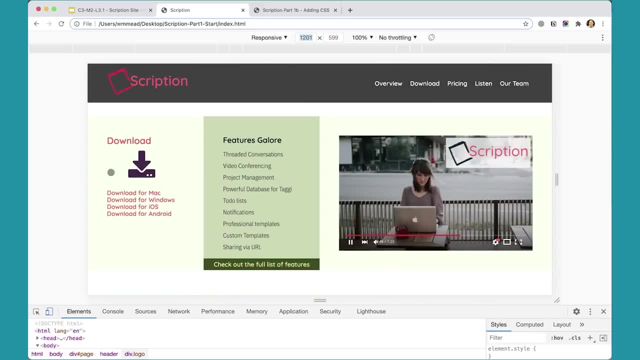 And so, since I've got some room, I might as well use it to give myself some white space, make the page a little bit easier to read, make it a little bit nicer. Down here again adding some room, 50 pixels padding around these things. 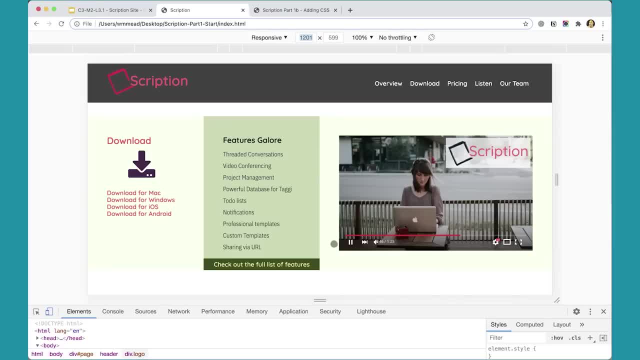 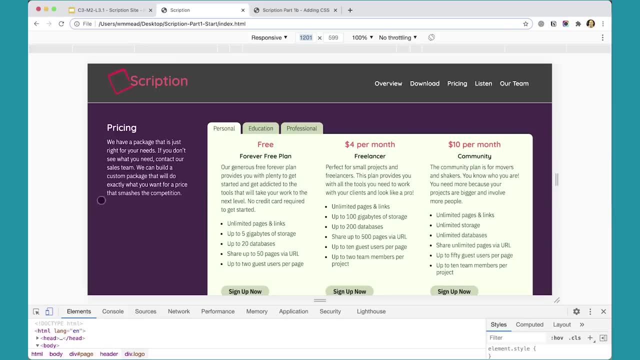 50 pixels padding around this element here. Give it a little bit of breathing room. Same thing down here. Now I've got some extra padding in here. Give it a little bit of breathing room. extra padding here To give it a little bit of breathing room. 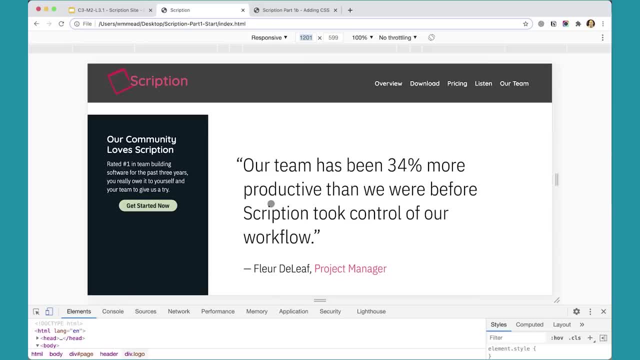 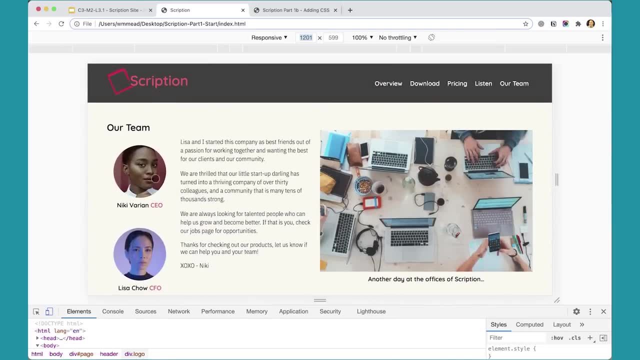 I've bumped up the sizing of this quote a lot. I mean really make it stand out. I've got the room now Might as well, right Down here. the team hasn't changed too much, just some extra spacing there. 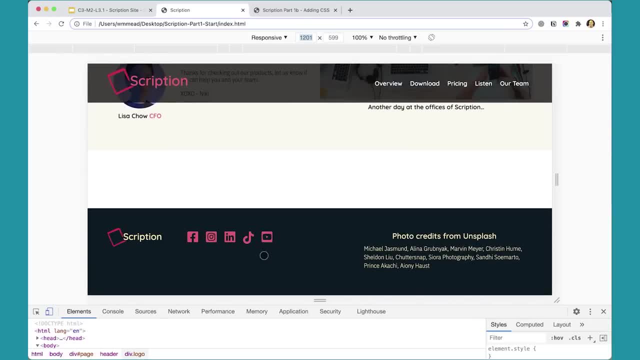 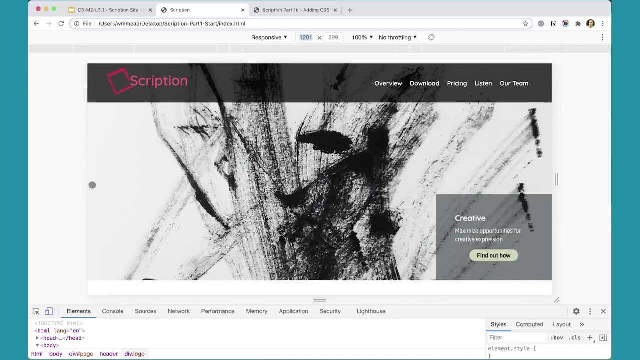 And then the footer got cleaned up with a little bit of extra room and kind of cleaning that up, And now we have the entire style of the entire page put into place And hopefully it came together. Okay for you, I recommend playing around with it. 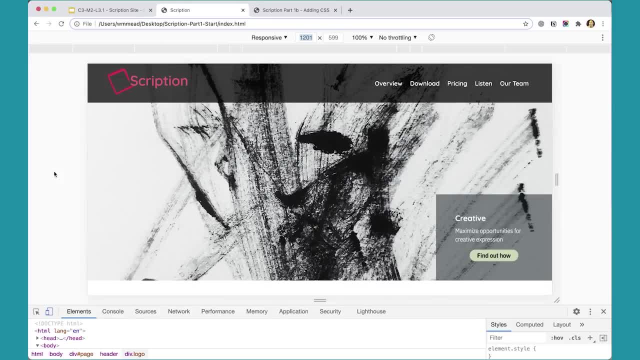 seeing what sort of different kinds of things you can do with it. You can always come back to my version. I will give you this version as something that you can download, So you can get my version anyway. So there's no reason why I shouldn't play around with this. 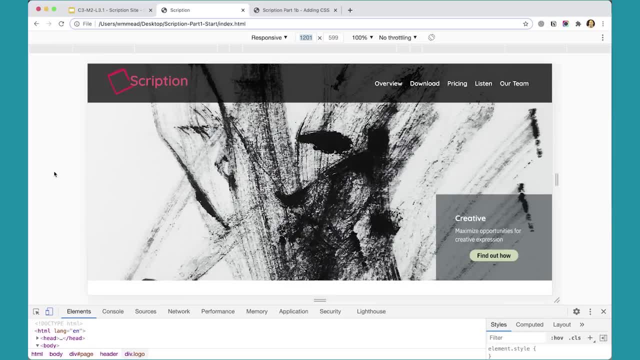 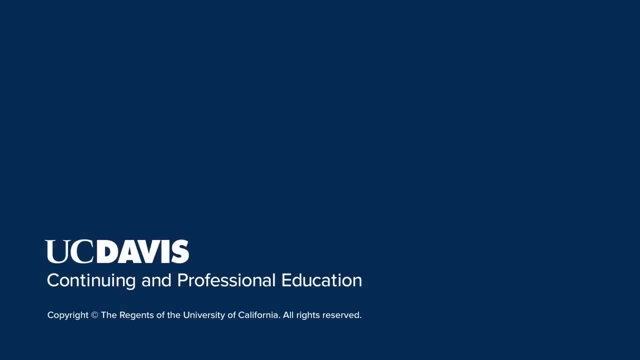 and mess around with it and come up with your own styling and see what you can do with it. It's always fun to do that. I'm glad to have you guys, So I'll see you again, Bye, Bye, Bye everyone. 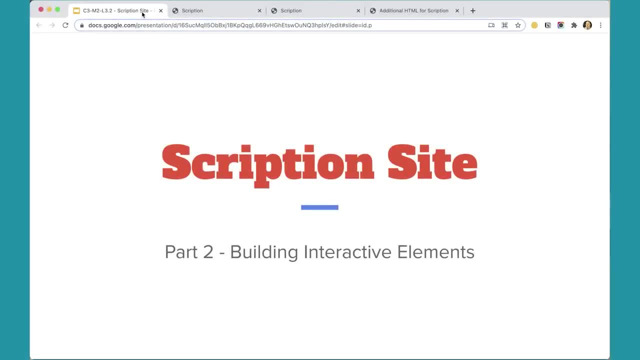 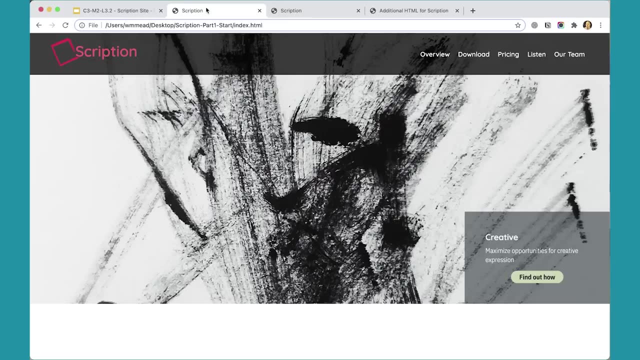 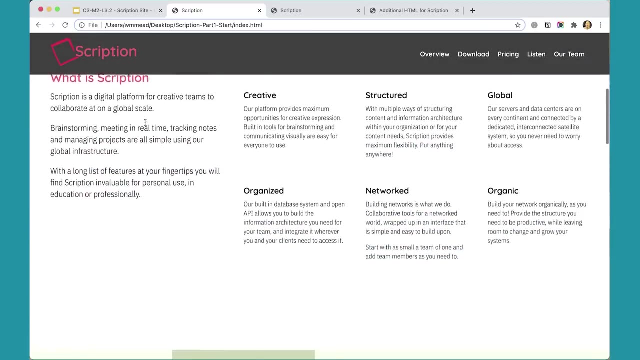 Subscription site. part two: building interactive elements. In the previous lesson we did the HTML and CSS to create this fictional web page for Scription for this fictional company And it looks really nice and I hope you like it And perhaps you did this. 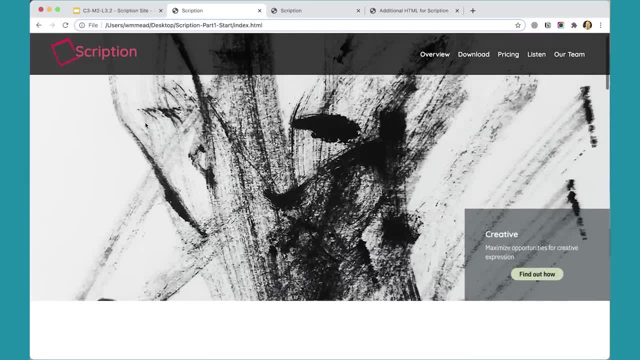 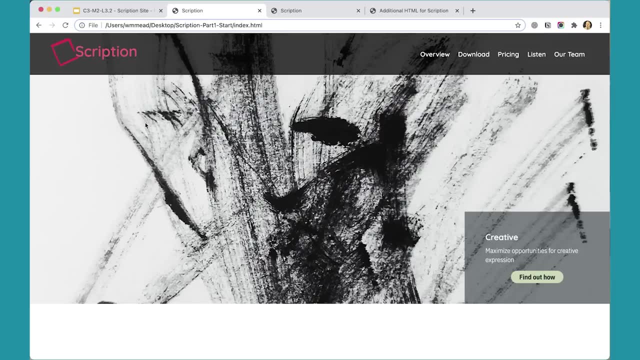 working with my files and either way, you've got a nice foundation on which you can actually build in some interactive elements. so this is your opportunity to show all the great things that you've learned in our javascript specialization and to do some challenges, to build some interactive. 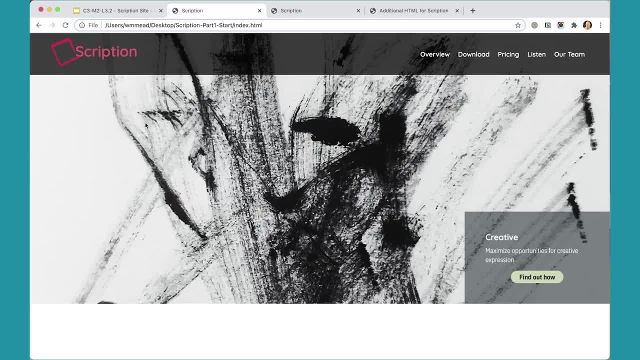 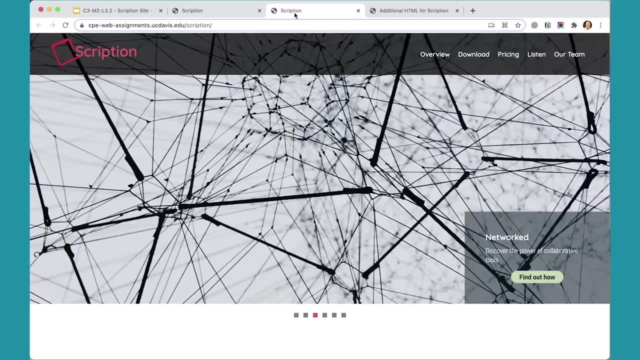 elements in here. so let's take a look at what some of these different interactive elements are. so if i come over to this tab here and i will provide this page for you so you can see what you're supposed to be doing here, i have description website with all of the interactive 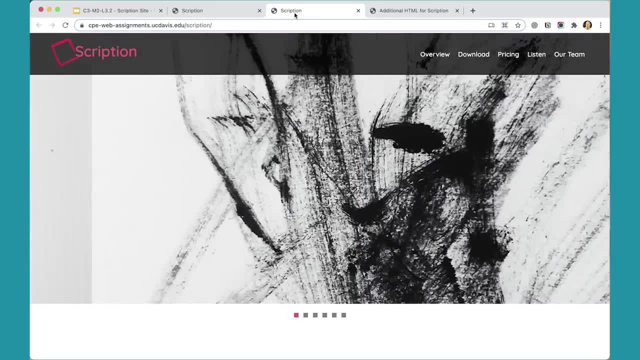 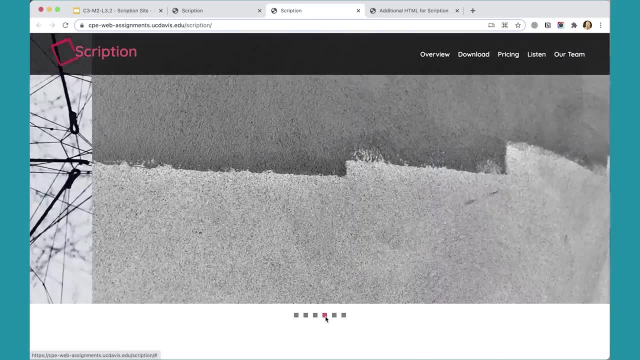 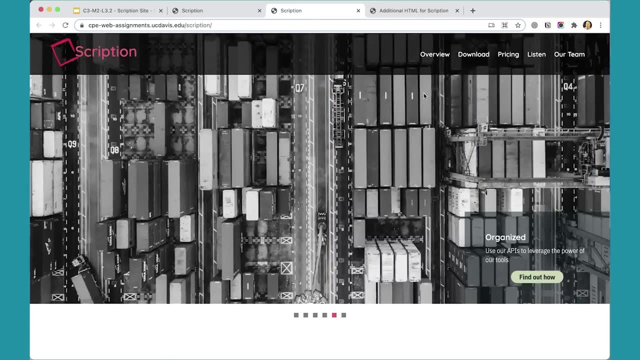 elements put in it. you can see that it's got a flex slider and it's running and doing its thing and it's functional. and you can click on the different links here- different pieces, different pieces here, this kind of stuff set that up. so that's all working, you'll. 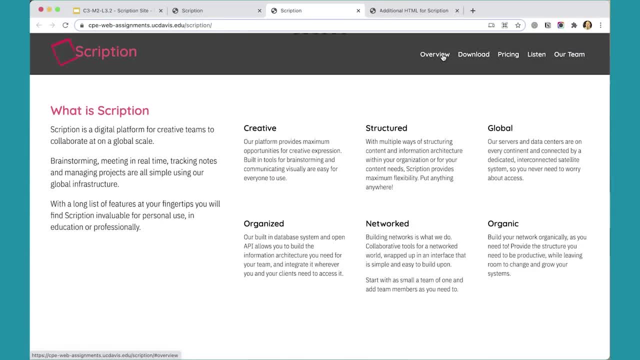 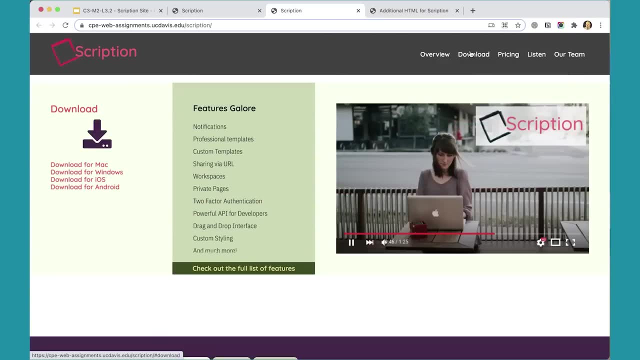 notice that i've got a nice smooth scroll script working here and it moves down to each section as we go down here. when we get down to the download section, this is really the the of all of the uh challenges. this is the toughest one, because this is the one that doesn't match exactly what. 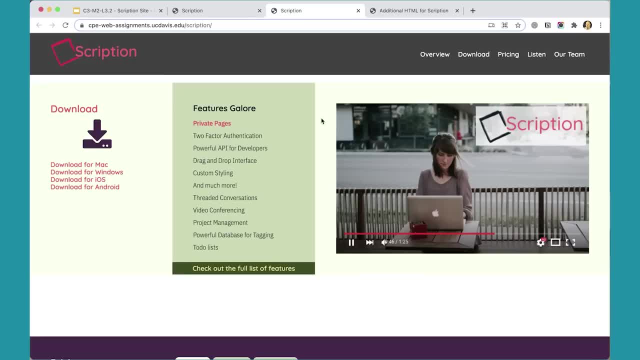 we've done in the other lessons. you're gonna have to figure out this one on your own, but these, uh, this list of items sort of moves up and pops into place and highlights the top item to give you a sense of all the features this piece of software has to offer. 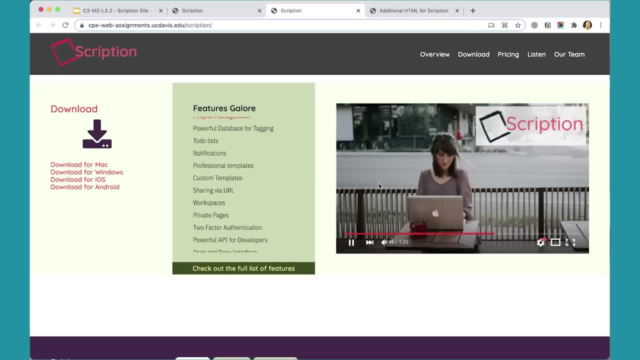 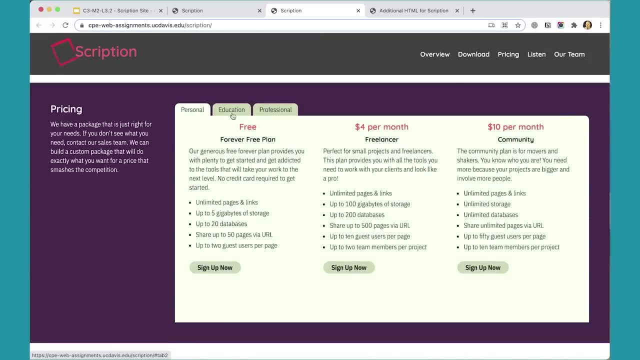 over here. this would be a video, but it's really just a picture of a video. no big deal. go down to pricing and sure enough you have tabs. you know how to make a tabbed interface. you can do it with jquery, you can do it with javascript. either one, i leave it up to you. 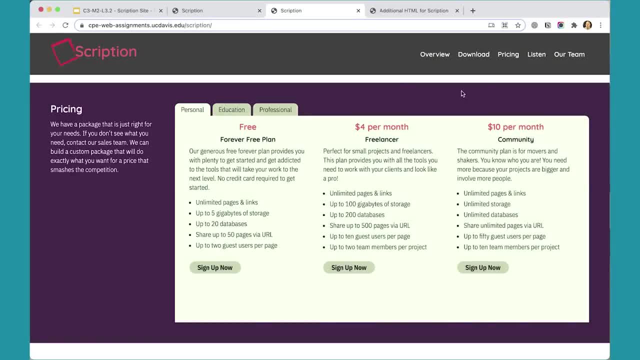 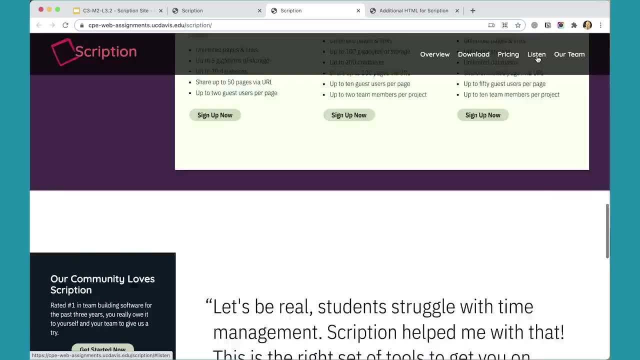 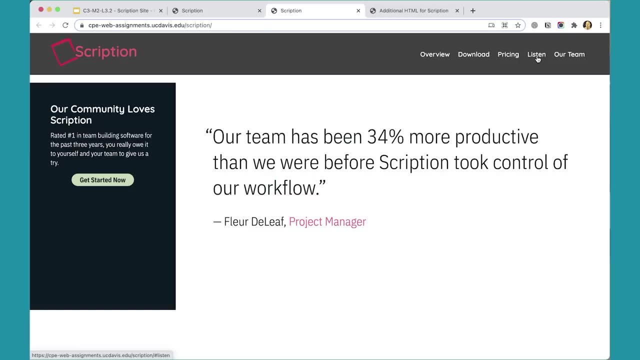 to choose which one you want to use. so tabbed interface down in the listen section you will see that we have the content rotator. you know how to put in a content rotator. we've done that. we've done that script. so it's your job to add all of these scripts together to make. 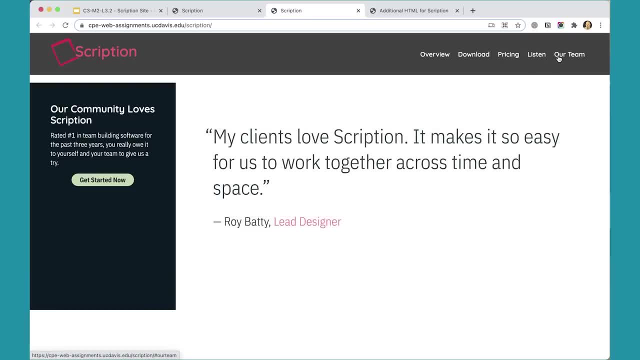 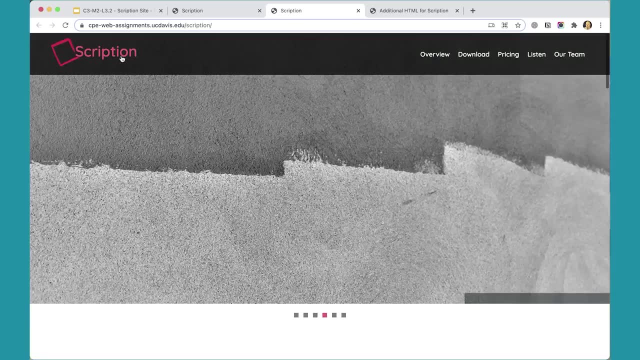 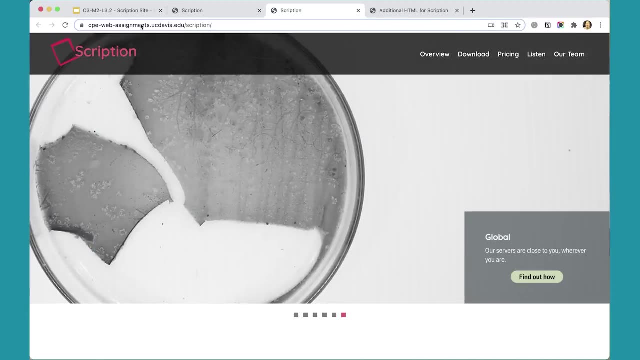 them all. look on, look right on the page. our team doesn't have anything interactive on it and the footer doesn't, but we can go all the way back up to the top of the page by clicking the logo. so these are all of the pieces for you to build in, and it should be pretty fun. so let's take a quick. 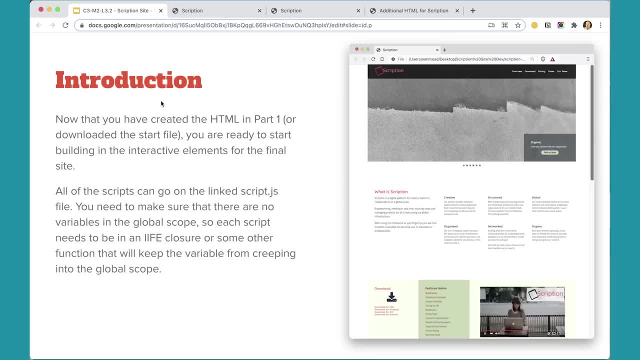 look over here at the challenges as they're laid out here. we've got all of that done and that's our introduction. we want to make sure you link to a script file, make sure there are no variables in the global scope, so each script needs to be in an iife closure or some other function that will keep the variable. 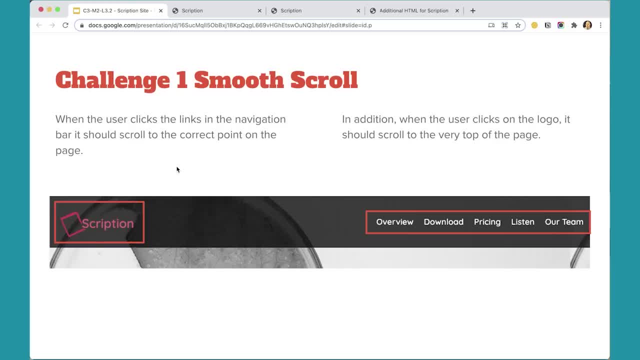 from creeping into the global scope. the first challenge is the smooth scroll. again, when the user clicks the links in the navigation, it should scroll to the correct point on the page. in addition, when the user clicks on the logo, it should scroll to the very top of the. 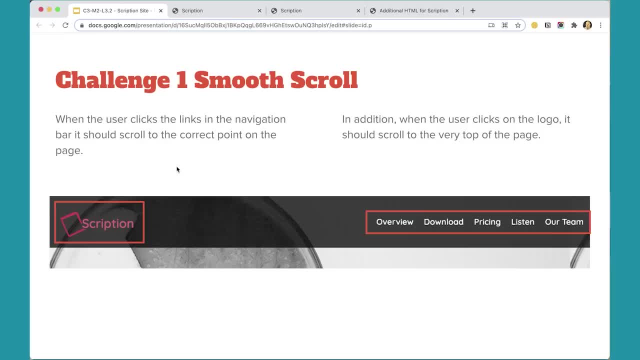 page. see, if you can figure it out. it's just a very small change from what we've done in the past with the, with the smooth scroll script. um, and it's really just the easy part of the scroll scroll smooth scroll script where it's scrolling down to the correct part of the page. we're not doing sort. 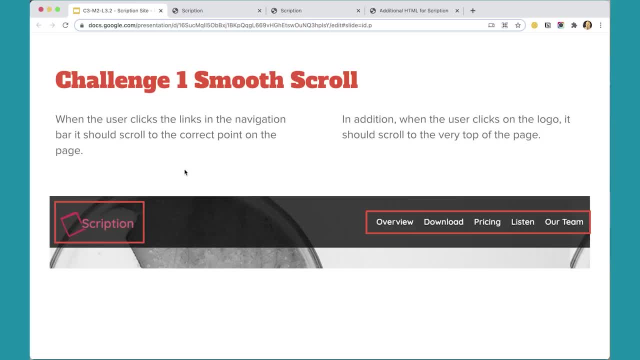 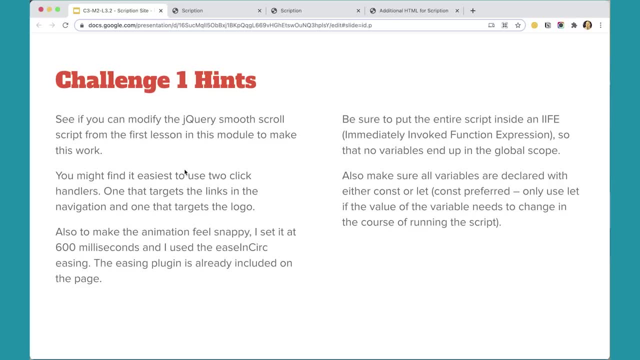 of any of the page tracking kind of stuff. it was much harder. so that's challenge one. some hints for this: see if you can modify the jquery smooth scroll script from the first lesson module to make it work. you might find it easiest to use two click handlers: one that targets the 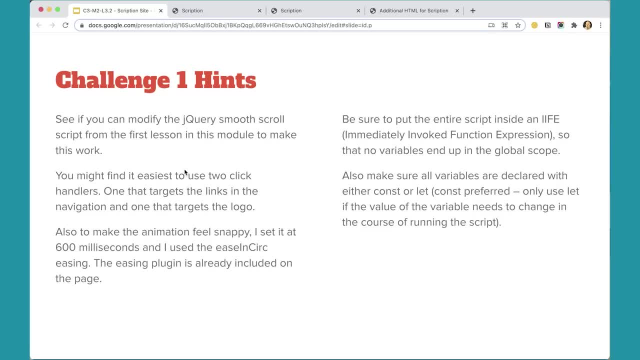 links in the navigation and one that targets the logo. i also made the animation feel snappy. i set it at six hundred milliseconds and i used the ease in button and the där you can, cuando dis вер, the opção se levantar para tirar, inserir o aplic. Titans noto a legendary 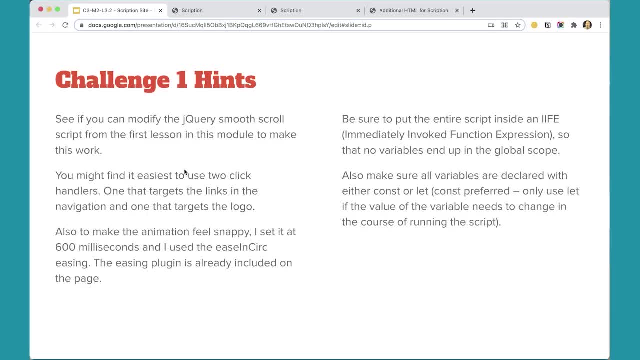 in circ easing. The easing plugin is already included on the page, so you don't even have to add that. Be sure to put the entire script inside of an IIFE immediately invoked function expression, so the no variables end up in the global scope. Also, make sure that all the variables 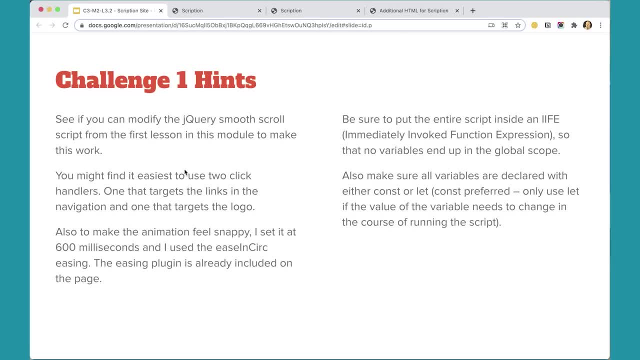 are declared with either const or let. Const is preferred. Only use let if the value of the variable needs to change in the course of running the script. And the way to do that is just to set everything to const and then, if it breaks, find which one is breaking and change that one to let. 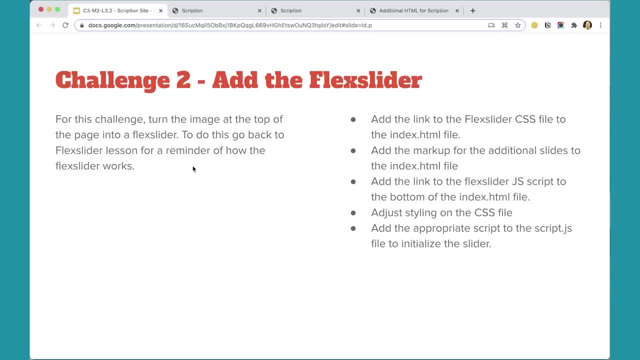 Usually it's const Challenge two: add the flex slider For this challenge. turn the image at the top of the page into a flex slider. To do this. go back to the flex slider lesson for a reminder on how the flex slider works. Add the link to the flex slider in the CSS to the index file. 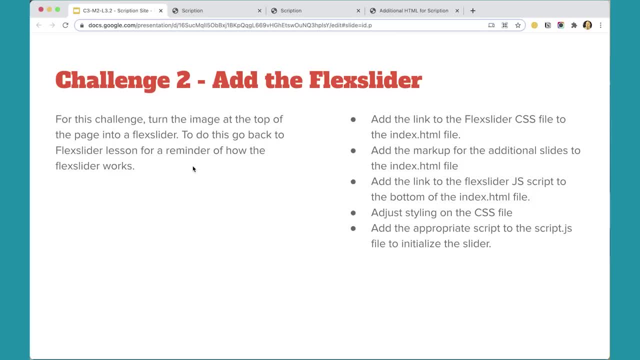 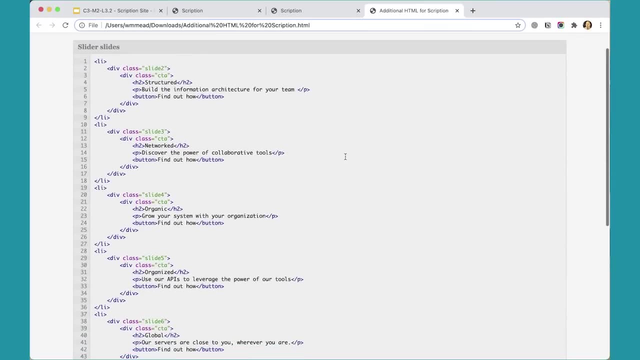 add the markup for the additional slides to the index file and, by the way, I've provided some additional snippets so that adding this markup will be easier. So here are all the list items that you need for the flex slider and I will provide this. 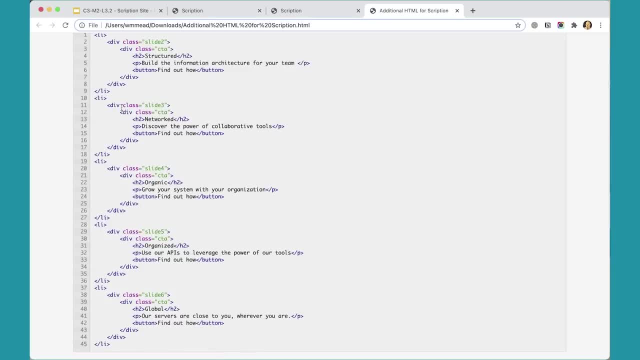 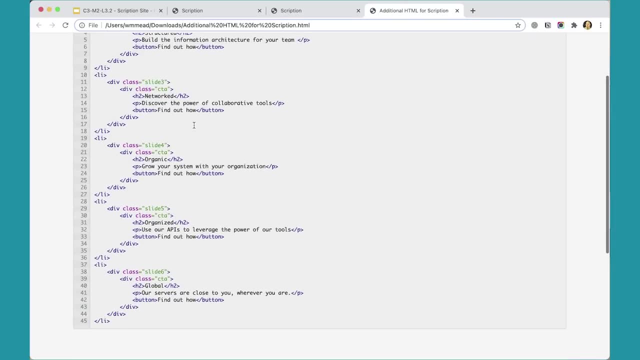 file for you so you can just paste this right in. You don't have to do a lot of tedious typing and all that kind of stuff, which is what I did when I made this. So I'm saving you the pain that I went through by providing you those snippets. 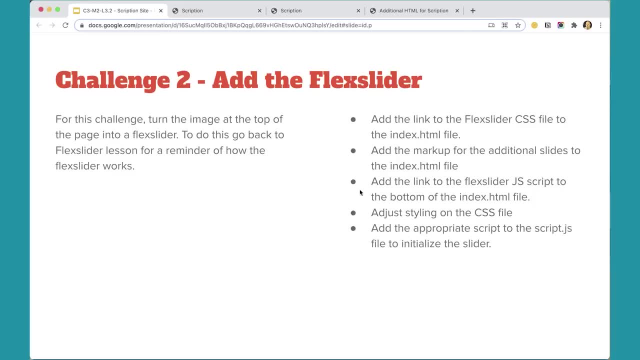 So you'll add the additional markup. add the link to the flex slider JS script to the bottom of the index file. I provided with this lesson again the download for the flex sliders files, so you'll need those in order to make this work. Adjust the styling in the CSS file and add appropriate. 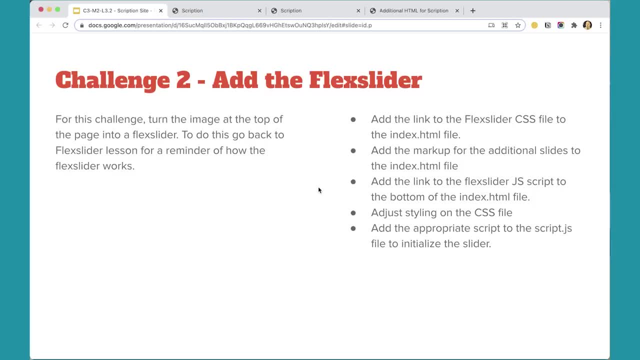 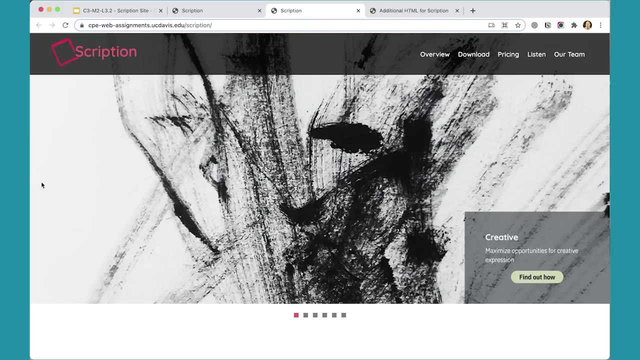 script to the JS file to initialize the slider, And I did modify the slider a little bit with some of the features that we saw in the other slider. Notice that I also got rid of the arrows that point left and right. That's a setting that you can, so 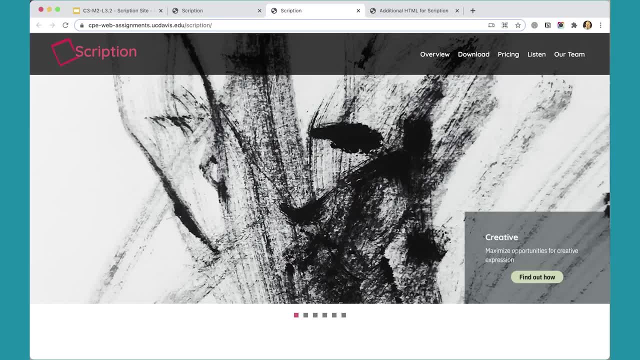 you can just turn them off by just setting it to false, And I got rid of that because they look okay on the desktop version, although they don't really go with the style of the site, but they really look terrible on the mobile version, So I decided I didn't want them anymore. 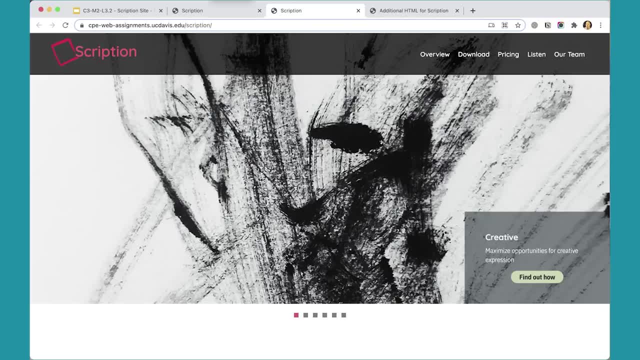 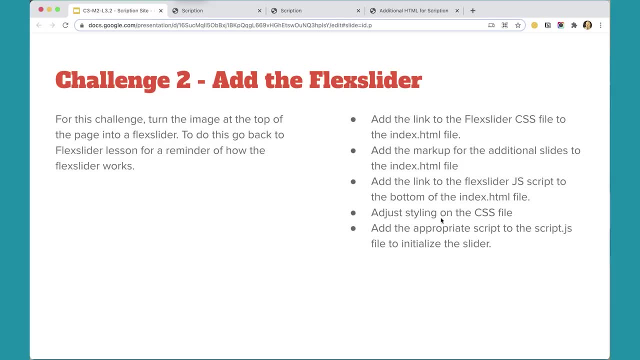 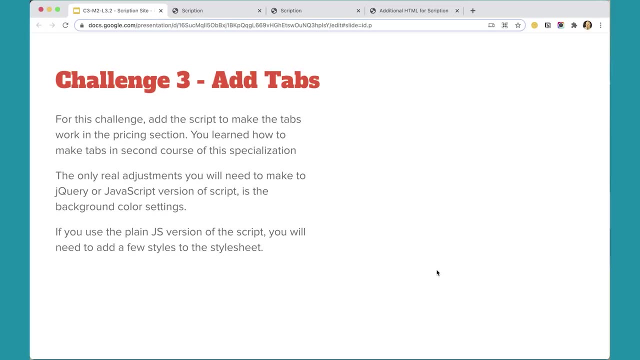 I didn't really need that particular item in there, So so I did that as well. Okay, great. So once you get the flex slider done, you can go on to challenge three. add the tabs For this challenge. add the script to make the tabs work in the pricing section. 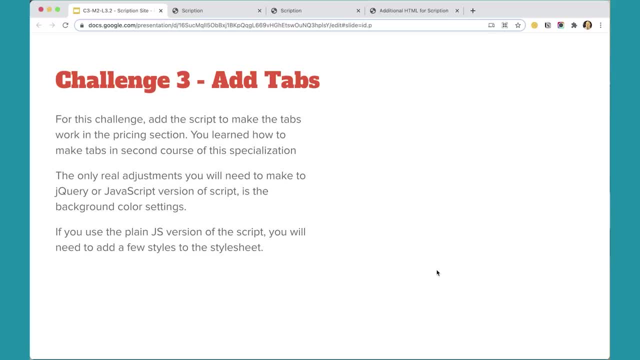 You need to learn how to make the tabs In the second course. you learned how to make the tabs earlier on in this course And in the previous course. the only real adjustments you need to make to the jQuery or the JavaScript for this version of the script is the background color settings. 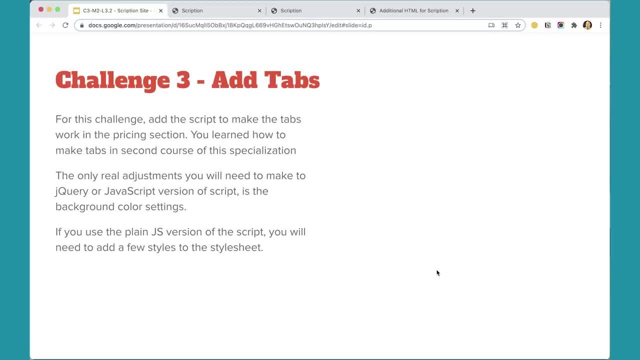 Other than that, it's really a copy and paste of the script. You could use the plain JS version of the script or you could add: um, you could use that version, But if you do, you'll need to add a few styles to the style sheet to make that version work And you can go back and 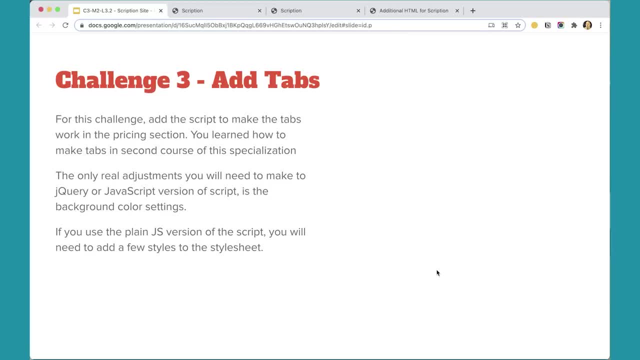 look at that version of that script to see what sort of styles you would need to add. So that's challenge three. to get that to work, Challenge four is to try out your product to see if it's worth using it. You need to try out your product to see what it's like to use it. 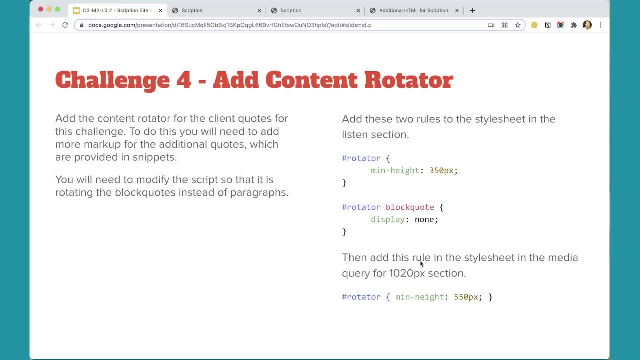 Challenge 4 is the Content Rotator. Add the Content Rotator for the client quotes to this challenge. To do this, you'll need to add more markup for the additional quotes which are provided in the snippets. You'll also need to modify the script so that they're rotating block quotes instead of paragraphs. 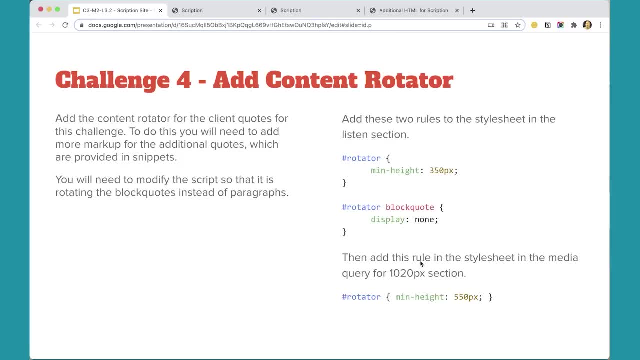 You'll also need to add these two rules to the style sheet. in the Listen section: Set the Rotator min-height and set the block quote to display none initially, so they don't come up showing at all. Also in the 1020 style sheet you'll change the min-height for the Rotator to 550 pixels. 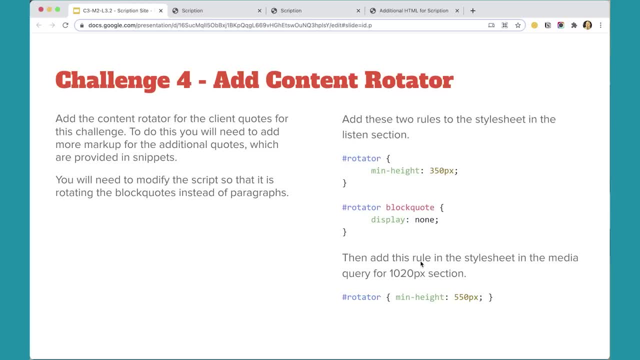 So once you get those sort of pieces in place, you can go ahead and work on the Content Rotator. You can pause this video here or come back to it to see exactly what's going on, What you need to do in order to get that to work. 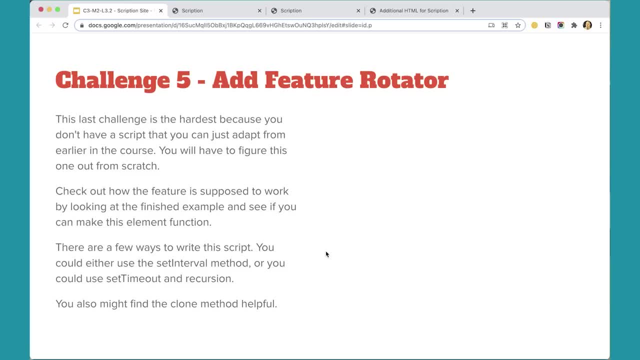 Challenge 5.. This is really the toughest challenge because you have not seen this one before, But you have all of the pieces you need in order to make the script work. So see if you can do it, See if you can figure it out from scratch. 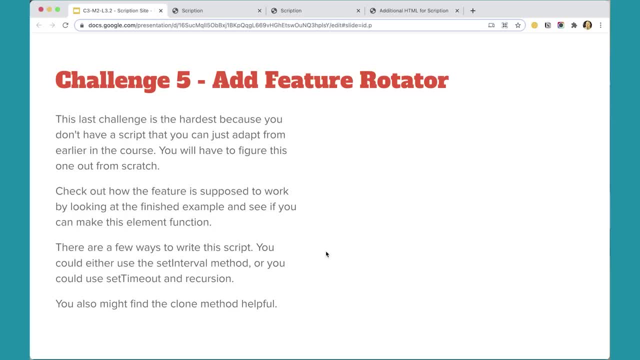 Check out how the feature is supposed to work by looking at the finished example. See if you can make this element work. There are a few ways to write this script. You could either use the SetInterval method or you could use SetTimeout in Recursion. 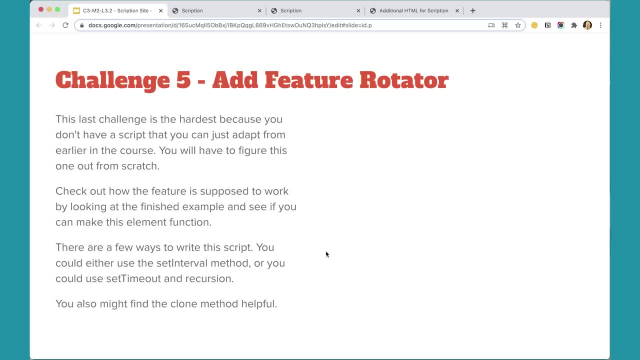 You might also find the Clone method helpful, And ultimately that's what I did. When the page loads, I make a copy of that unordered list that sort of is rotating into place, I clone it and put it at the bottom And then I move them both up together. 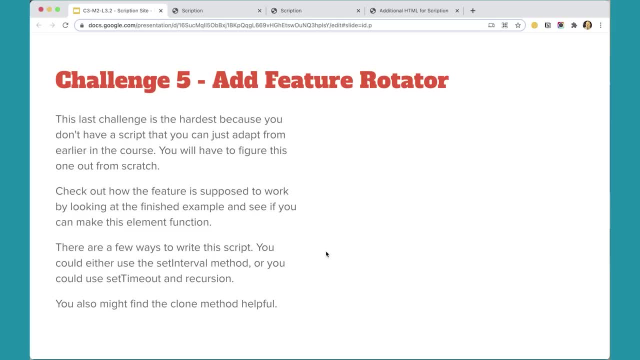 When the top one moves off the screen, I remove it And then clone it at the bottom. This is very similar to what we did in the slider script that we wrote- our own slider script that we wrote with jQuery, So it's a very similar technique. 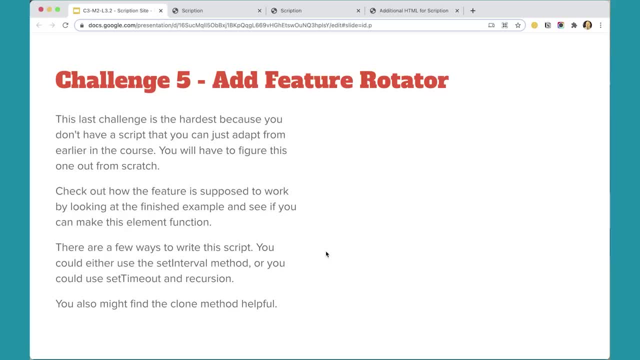 See if you can make it work And with that I'll let you go forward and see what you can do with this And I hope you post on the discussion boards what you found successful and help out others who are working on this project. 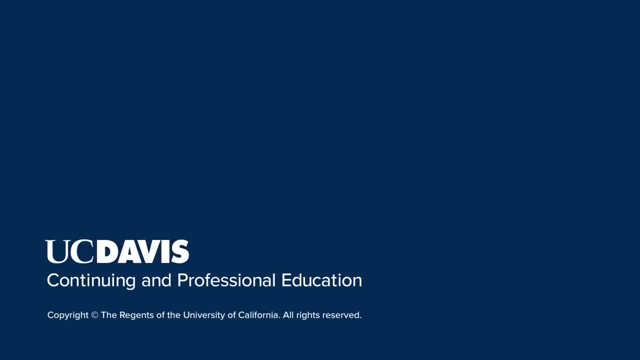 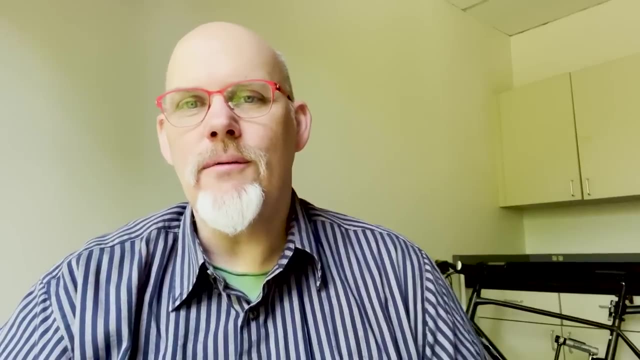 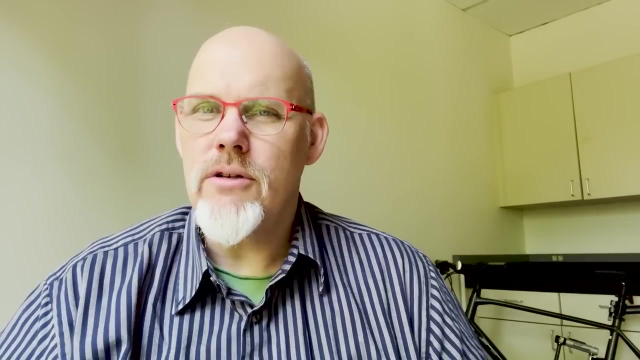 Hopefully it's a lot of fun. Hello and welcome to the third module in our third course on JavaScript. In this module we're going to introduce objects And we'll do a lot of practice with them so you can get good at the syntax and get comfortable with working with them. 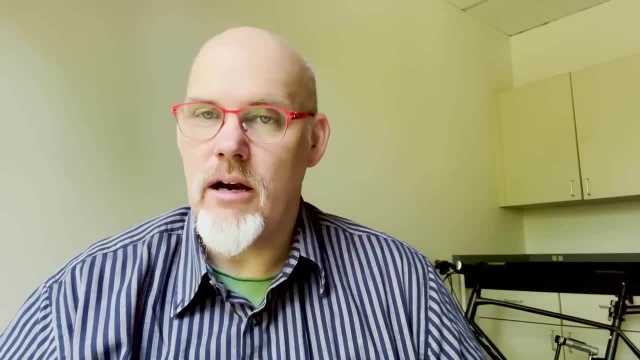 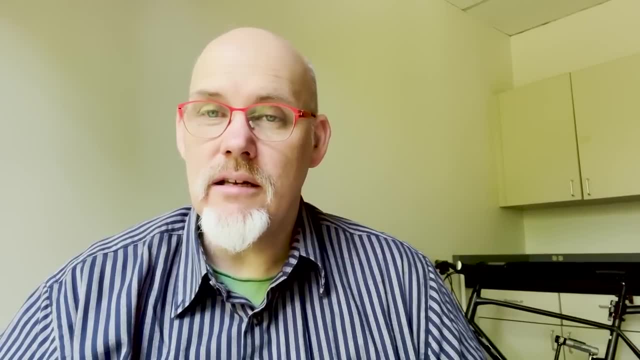 Plus, we're going to introduce a game that we're going to work on in our fourth module and see how we can take a more complex script and break it down. It's really interesting content And I think you're going to get a lot out of it. 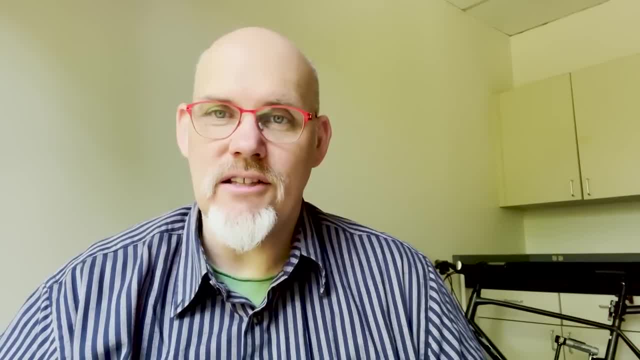 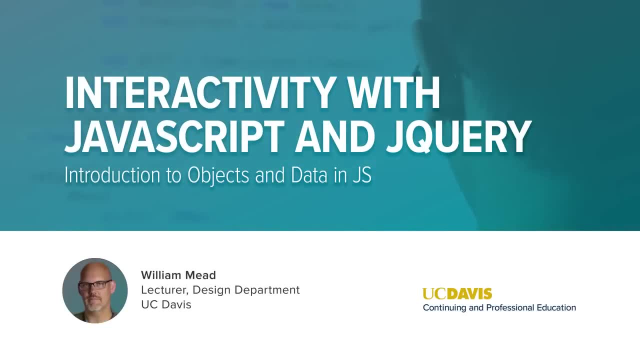 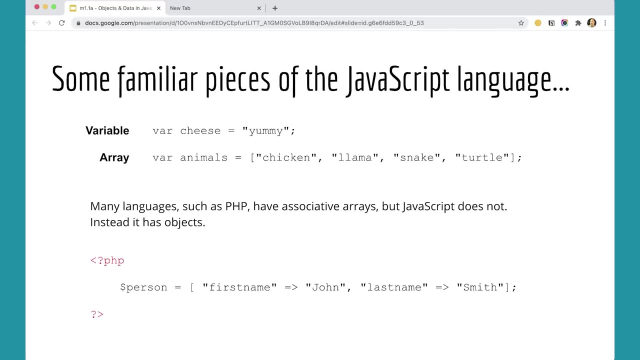 So I look forward to doing it with you. Let's get started. Objects and data in JavaScript. Let's talk about a few of the familiar pieces we have with the JavaScript language. You're already familiar with variables. That's a data structure that can hold a variable. 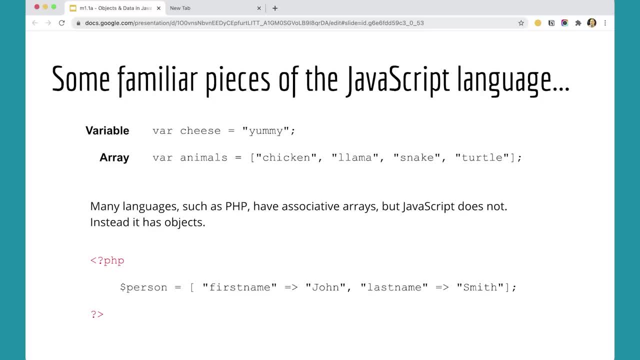 We have var cheese and it can hold a value like yummy. Or we have an array. that's another data structure that we're familiar with And an array can have. here we have var animals and it can have several animals in the array. 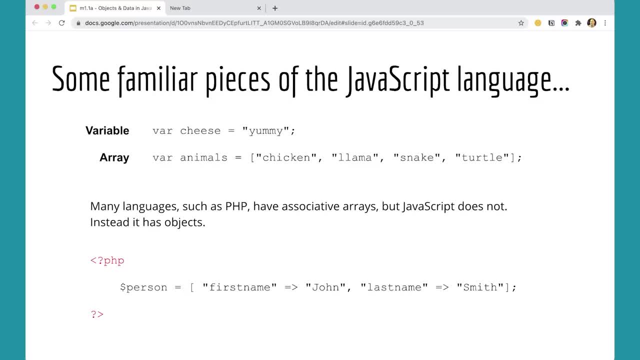 So we're familiar with those in JavaScript. One thing that JavaScript does not have is associative arrays. Other languages, some languages like PHP, have associative arrays And an associative array, as seen below. here is an array that has a key value pair for each element of the array. 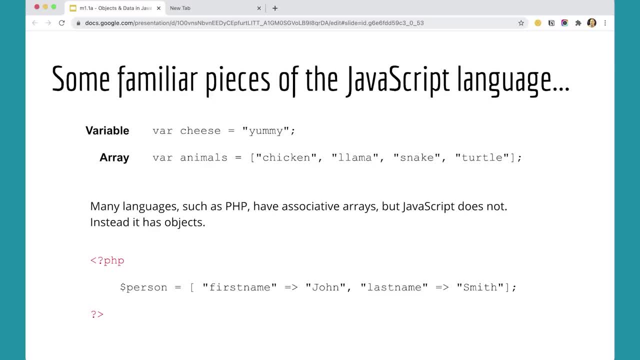 So down below here we have a variable person And in PHP you recognize a variable because it starts with the dollar sign. But we have a variable person and it's an array And in the array we have key value pairs. 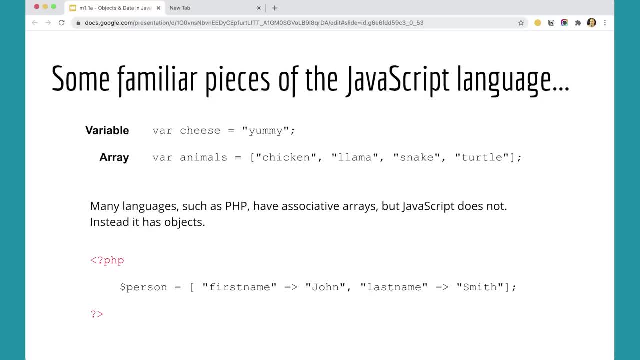 The key is first name and the last name is. And then there's the first name, value, which is John, And then we have another key, which is last name, which has the value Smith in there. Well, we can do the same thing with JavaScript, but not with arrays. 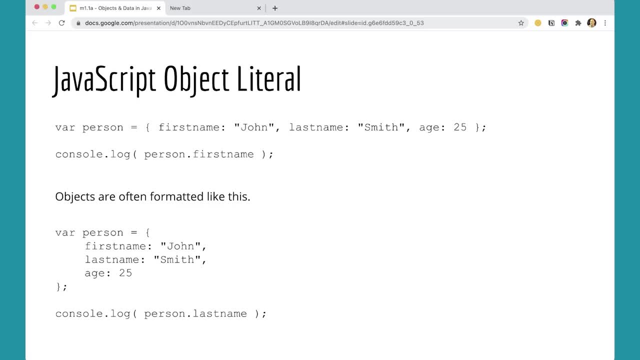 Instead we'll use objects. This is the object literal in JavaScript. Here I have a variable person and it's assigned an object, And the object consists of key value pairs. Sometimes these are referred to as members and sometimes they're referred to as properties. 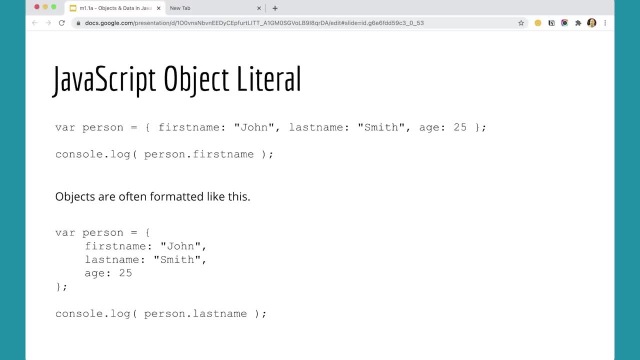 The first name property of person or the last name property of person. And then first name has a value, which is John, and the last name has a value which is Smith, And age is another property with a value of 25.. 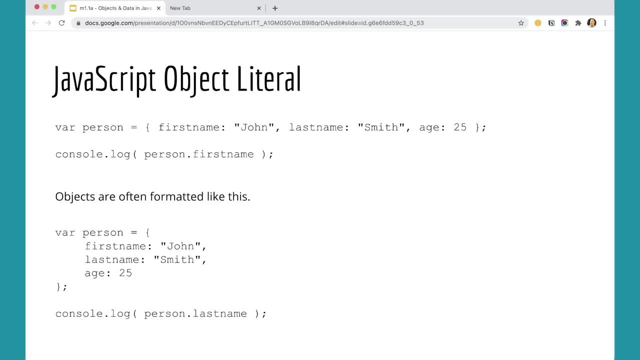 And the way you would access these in JavaScript is typing the name of the variable person, and then a period or a dot, and then the key, the property first name, And that will give you the value. John, Frequently you'll see objects organized like this: 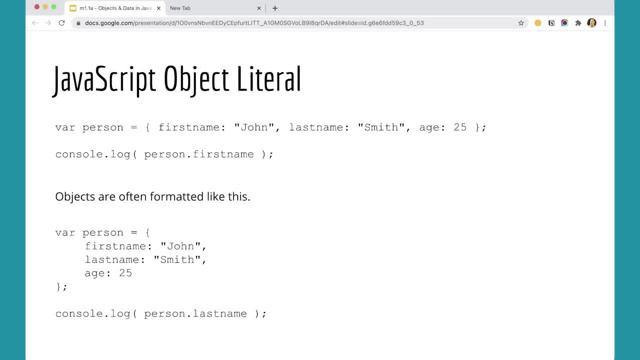 var person And then you'll have the first name on its own line. Each member of the object, each key value pair, each property will have a line inside the object And notice that first name doesn't have quotes around it, but John does. 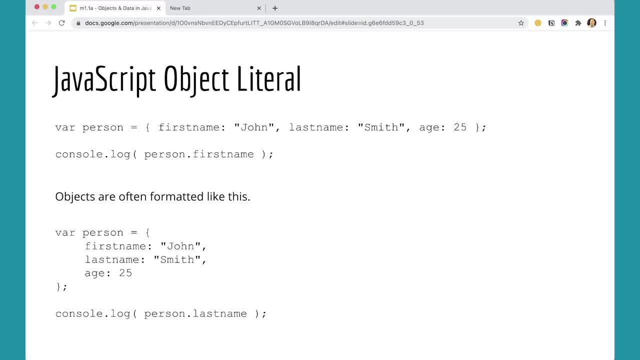 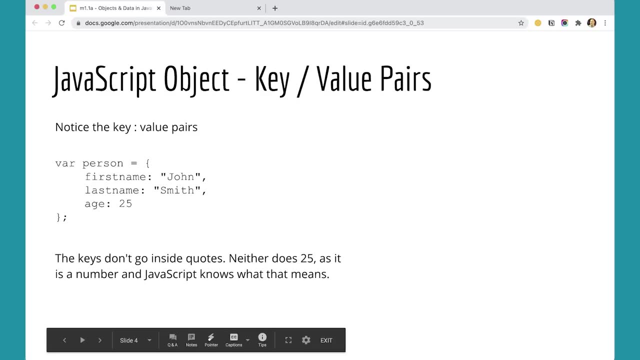 And this is how you'll frequently see objects listed in JavaScript. This is in this sort of format because it's easier to read. Now notice here again. I'm going to point this out because this is really important: The key in the object first name does not get quotes around it. 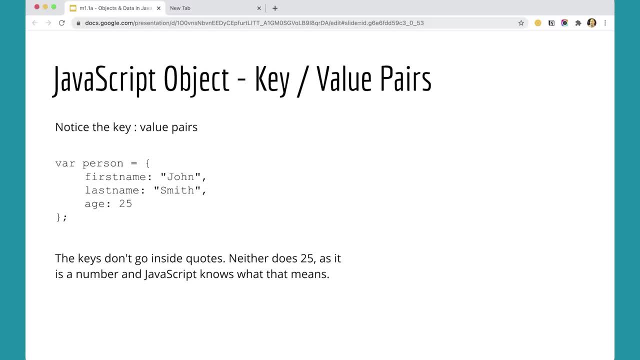 But the value does, Unless the value is a number like 25.. Here we have age 25.. And JavaScript knows what a 25 is. The other thing to notice here is that each key value pair is followed by a comma, except for the last one. 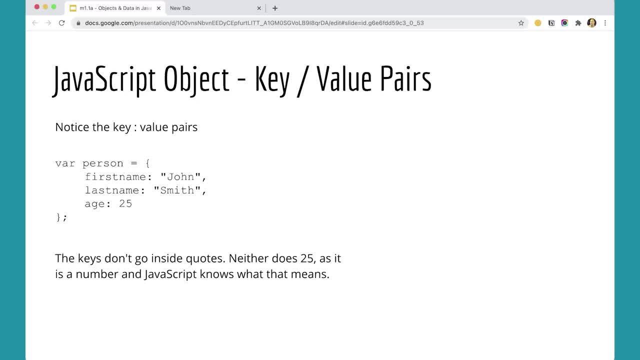 And that's really kind of important as well. So you'll have key value pairs and one on each line. one key value pair on each line, followed with a comma. Now, it's really important to get in the habit of actually typing this. 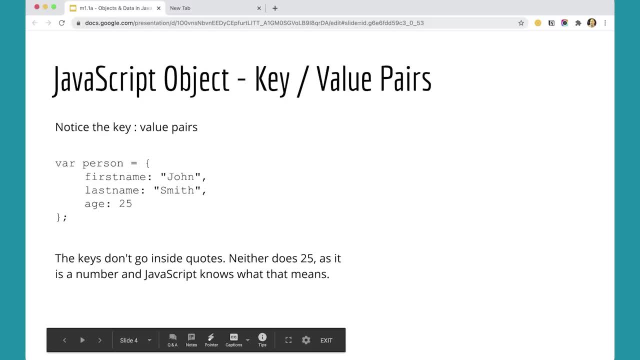 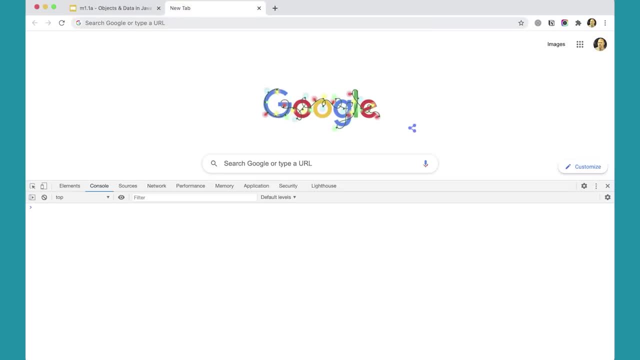 And to do this now, just to demonstrate, you could come over to a new browser tab. open up, choose Inspect. right-click and choose Inspect and open up your console log here. You know, you get to the console log here. 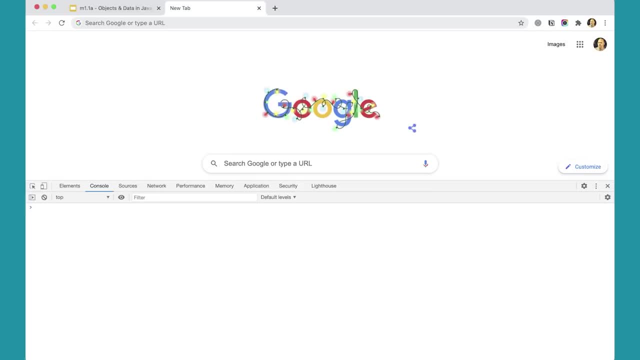 And then practice typing this: var person equals quote And you can see I had typed this before so it's already in here. But I've got first name Jose And that goes in quotes And it's really important to type this and to do this. 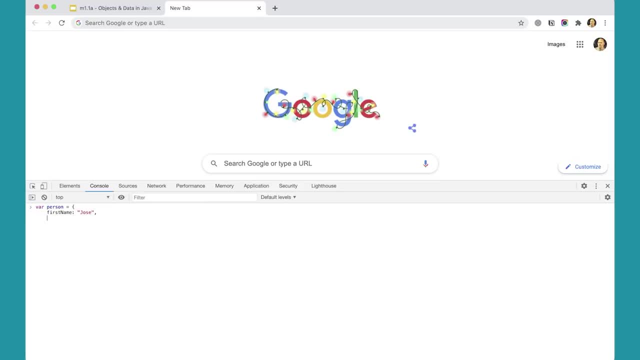 even with these very basic exercises, just because the way you learn JavaScript is by actually typing it. You're not going to really learn it unless you actually type it and really you know, see and feel and get some muscle memory in or around the actual syntax. 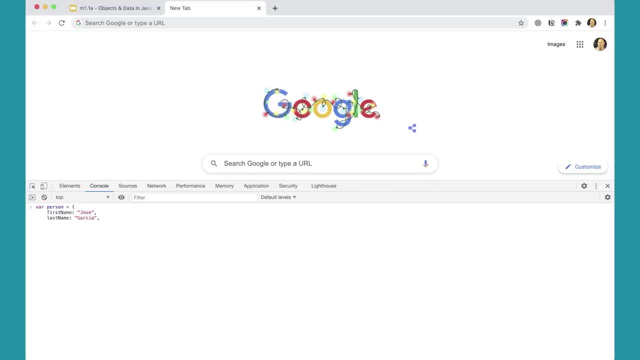 And then we have a comma there And then we'll add age 25 or whatever you want to put in for an age, And remember that one does not get a comma, We just close the object And that object has been defined. 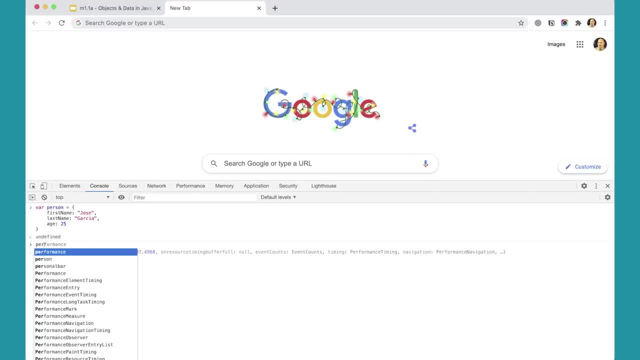 And now I could access personfirstname And you can see it even fills it out for me. I can press Tab and it'll return, Jose, And that's great. So you want to practice this as much as you can and get used to using these data structures. 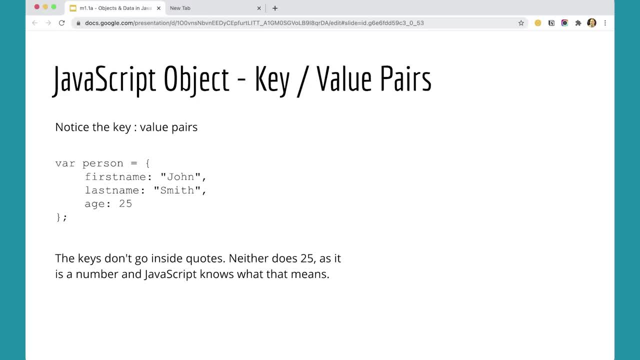 One more thing about objects before we close out this video Is that you can also create an object like this. Here I have person, a variable person, and I've assigned it using the new keyword new object with a capital O, And that will create a new object. 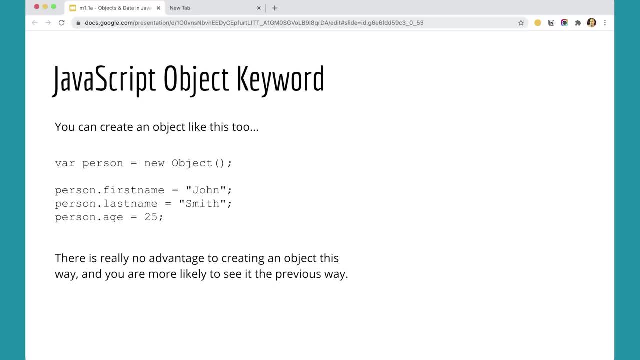 And then I can create members of that object very easily by just typing person dot and then a key like first name, and then assign it a value like so, And you can create objects this way, But it's much more common to see them created the other way. 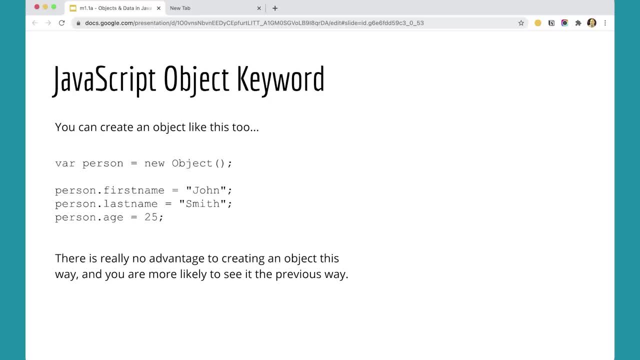 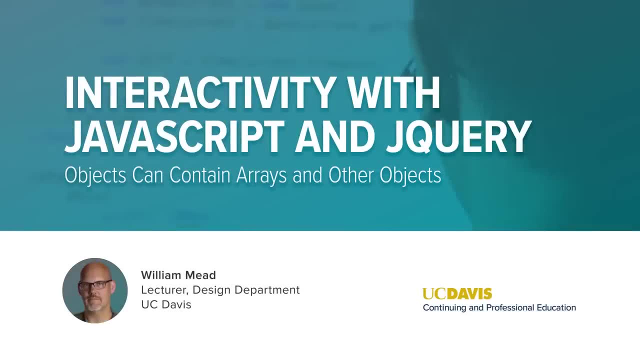 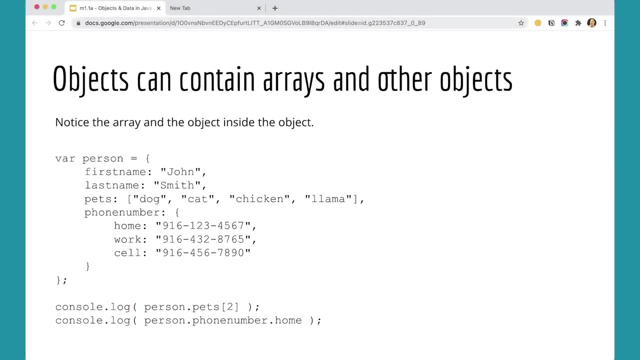 using the object literal. It's shorter syntax, It's a little bit easier to follow, But you can create objects this way as well. The object data format in JavaScript is very flexible, because objects can contain arrays and other objects. So here you can see we have an object called person. 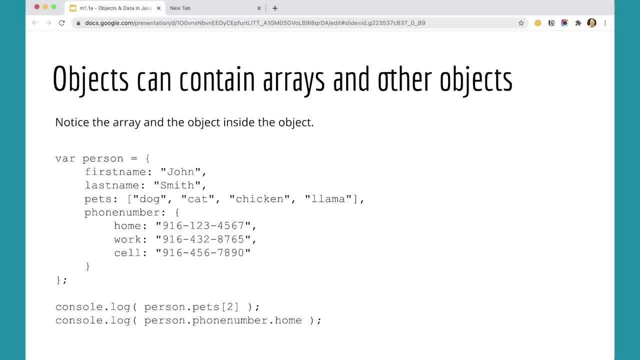 And we've expanded it a bit, So it has first name and last name, But it also has an array for pets. So pets is holding a value. that's an array. It has another object. as a member of this object, The phone number is an object. 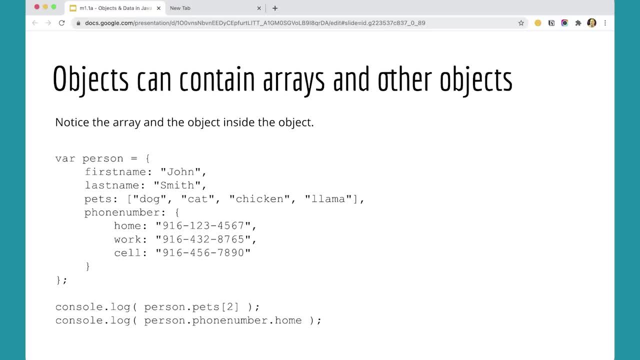 So it's an object inside of an object And inside phone number it has its own key value pairs And then we can access these different values through similar methods that we used before down here. So I really recommend typing this out and seeing if you can get it to work exactly the way this works. 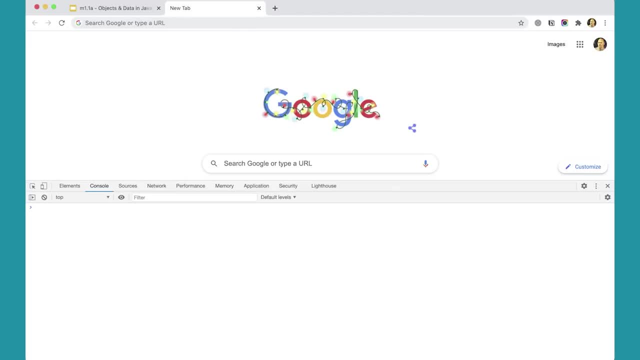 I'm going to do that over here And you're not going to have to watch me type it out, because that's kind of painful. I'm just going to paste it in here. But you can see, I've created this object And now I could access elements of this object. 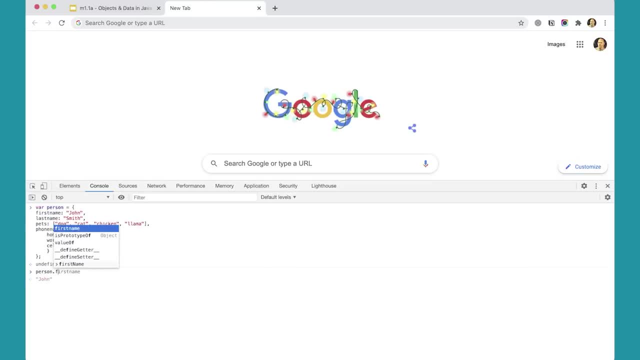 by doing person dot first name Or person dot pets, square bracket two will get me a chicken, Zero one, two, So that gets me the chicken. Or I could do person dot phone number And then within phone number I could have work. 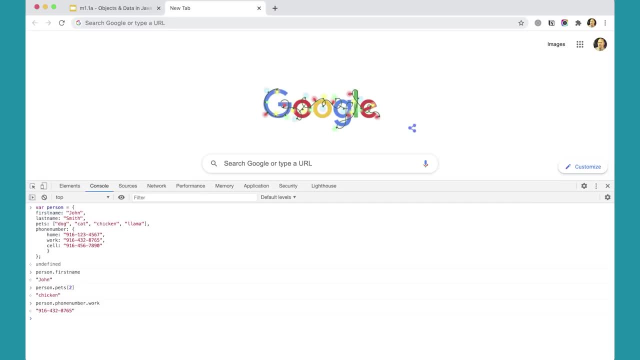 And that will get me the work Work phone number So we can access all the data inside of this object. You can even update data very easily with this, And we'll talk more about this later, But it's possible to update data. 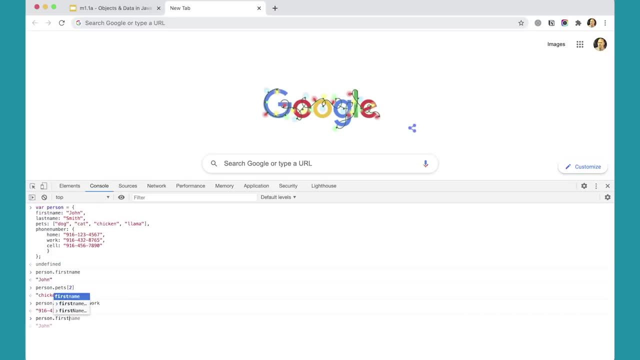 If I did person dot, first name equals Jose. That needs to go in quotes, Like: so You can now see that person. If I just do person, You'll see I get the whole object here And that first name is set to Jose. 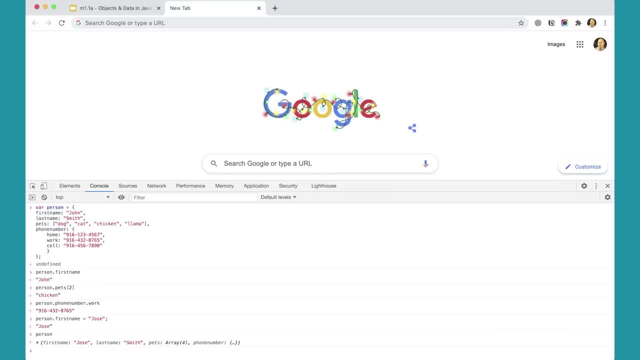 So we can actually work with the data inside the object And we can update it. Or we can access the data that's inside the object And the object can have other objects, It can have arrays- All kinds of fun stuff can be done. 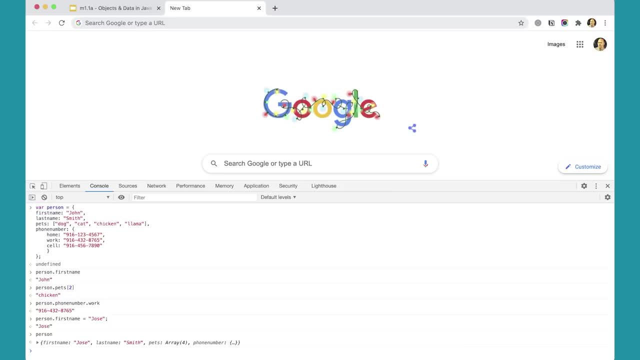 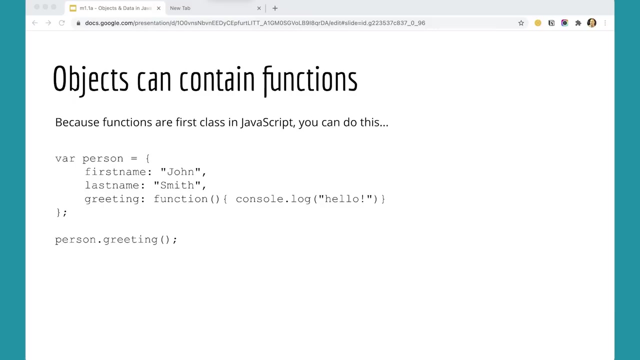 All kinds of fun stuff can go in there, And that's a really important thing to understand about objects as a data structure. They're very flexible And very useful for working with in this way. Another thing that's interesting about objects is that they can contain functions as one of the values of one of their properties. 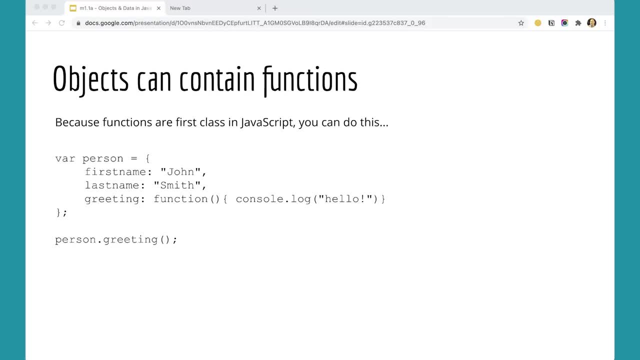 And that may seem like a weird thing, But remember, in JavaScript functions are first class, So wherever you can put data, You can put a function. So here you can see, I have an object for a person with first name and last name, And then I have a greeting. 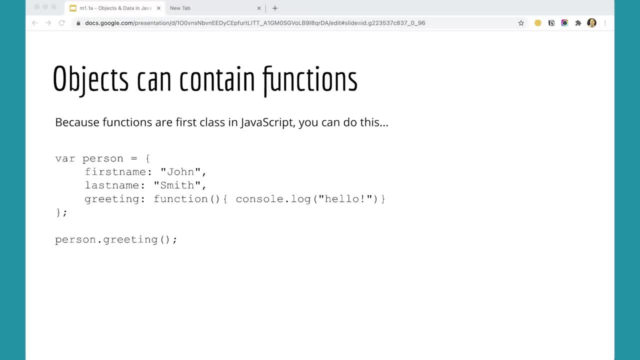 Which is a function, Which has a value, which is a function And the function. all that function does is console log out, hello, It doesn't do anything very interesting, But we can access that value. We can access that function by doing person dot greeting. 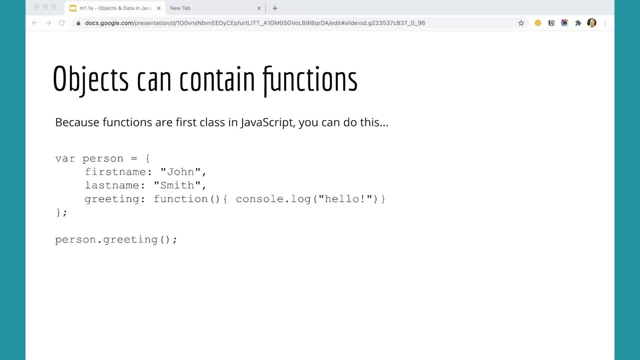 And then putting the parentheses after greeting After that property, It will run that function. that's in that assigned to that greeting key there. So let's do this really quickly, Because this is kind of interesting If you come back over here to your tab. 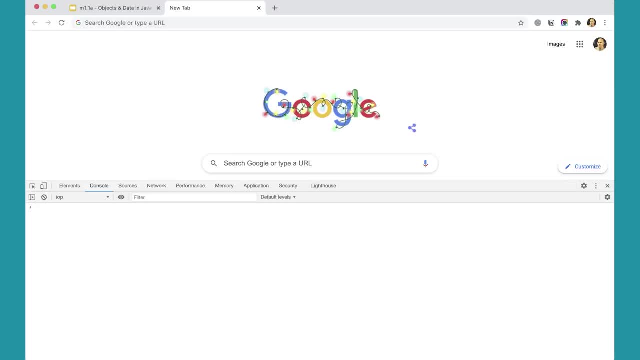 We can clear out the console here And I'm just going to paste this in Just so that it's there and it's all done. But now I can do person dot greeting And you can see I get hello. So it's actually running this function. 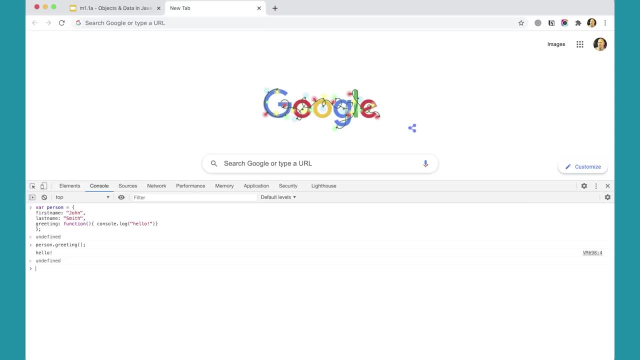 This anonymous function that's assigned to greeting here. And remember when we put a function as a member of an object, This function, this hello function, belongs to person. Remember what we call that. That's called a method, So it's really kind of amazing. 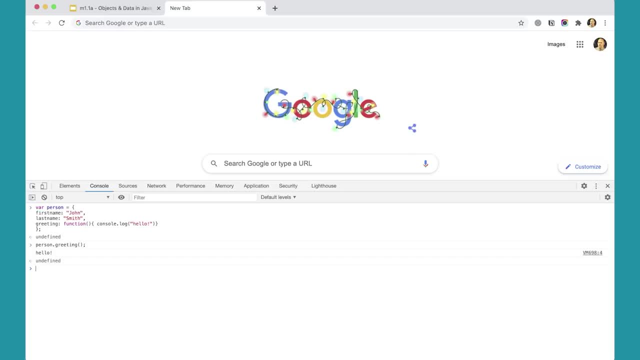 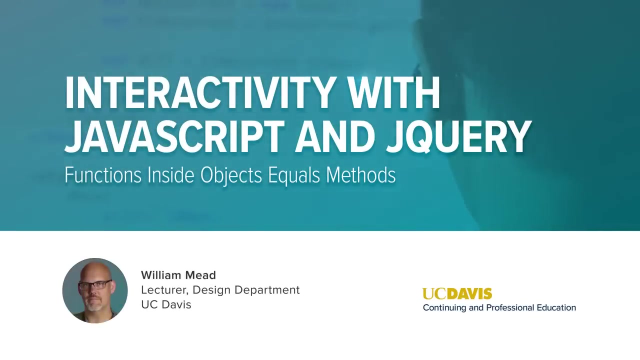 That you can assign a method, Create a function, Create a method that belongs to an object And then access that method through the object, Like this person dot greeting, And that's a really cool feature of JavaScript and objects. Let's take this idea a little bit further. 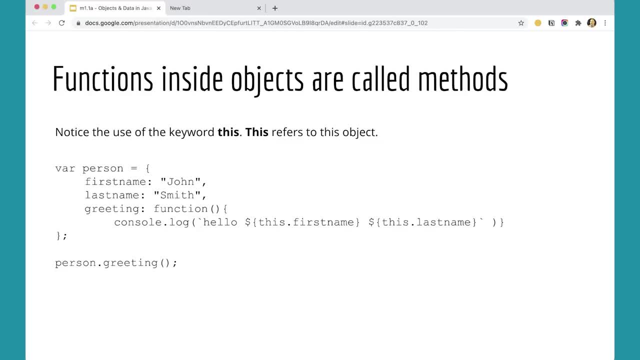 We can put functions inside objects, Which again are called methods, But also we can use the this keyword to reference other objects Or other keys within the object, And that can be pretty handy. This can be pretty helpful from time to time. So here we have person. 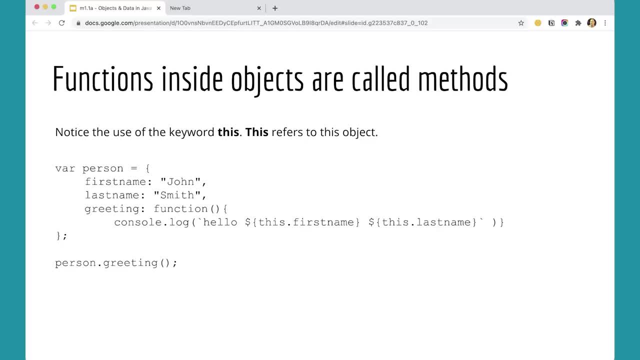 And we have a property called first name Which has a value John, A property called last name Which has a value Smith, And a property called greeting that holds a function And this function is going to just do a console log, But the console log is going to say: hello, this dot first name. 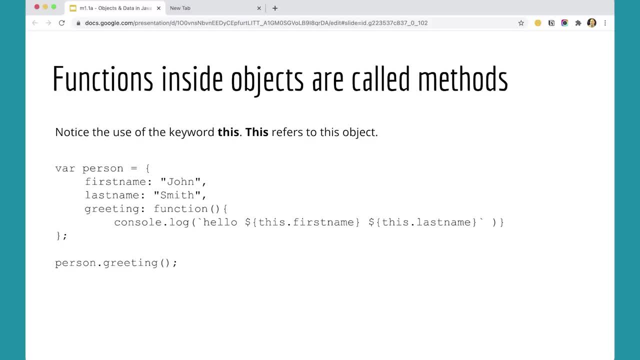 So that's going to go into the first name property And get the value and put it there. And this dot last name. So that's going to go into the last name property And get its value and put it there. So we should get hello John Smith out of this. 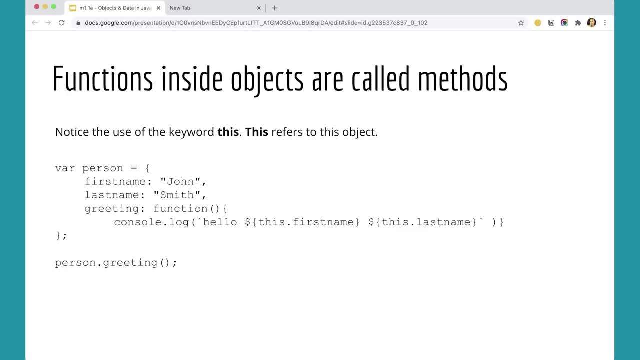 And the this keyword can be somewhat confusing in JavaScript, But it refers to this object, This person. That's the context in which this makes sense here. So let's give this a try over here And again, I'm just going to paste it in. 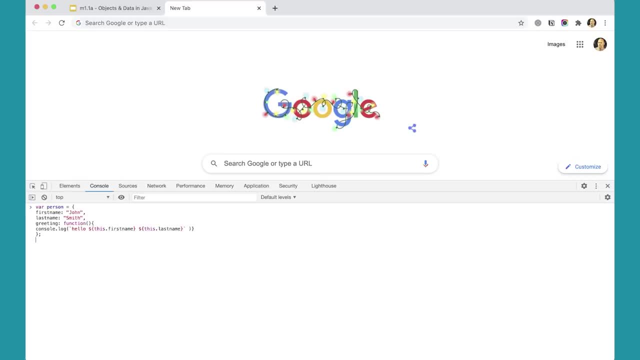 You're going to have to type it, But I've got. Let's see if I can tap This in a little bit, Make it look a little better. There you go. So I've got that in there, And now, when I've defined that, 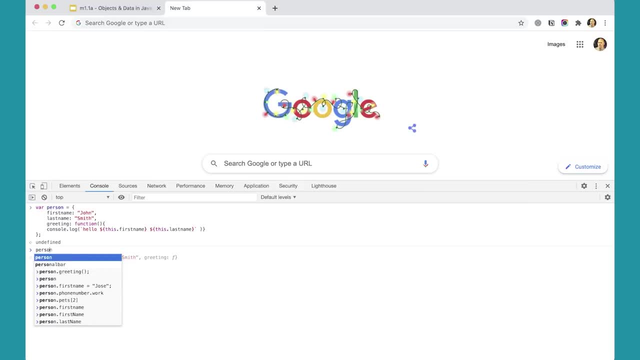 I can do person dot greeting And it will say: hello, John Smith. So this is referring to this first name And this last name, And remember that this is a keyword here In JavaScript, So that's important. The next thing to talk about is the object constructor. 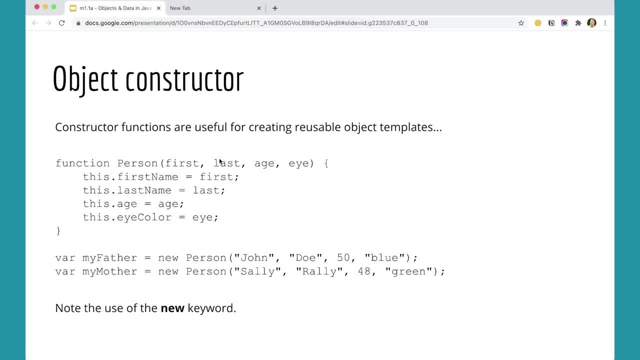 This will push our objects even further, into something even more useful, And what an object constructor does is it creates, It uses a function to create an object That could be like a reusable template That you could use over and over again. So here, if you look at this, 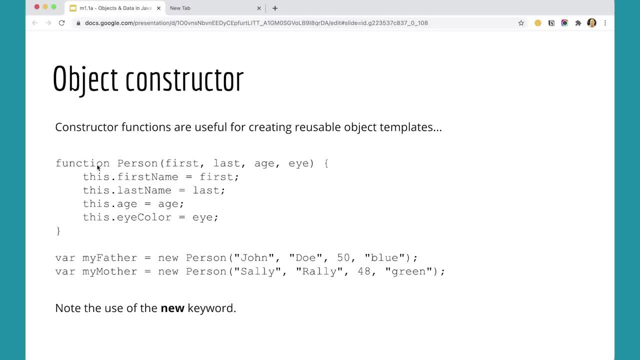 What we have here on this screen. We have A function person And when you create Constructor functions, The standard is to make the first letter of the name of that Constructor A capital letter, So it's person with a capital P. 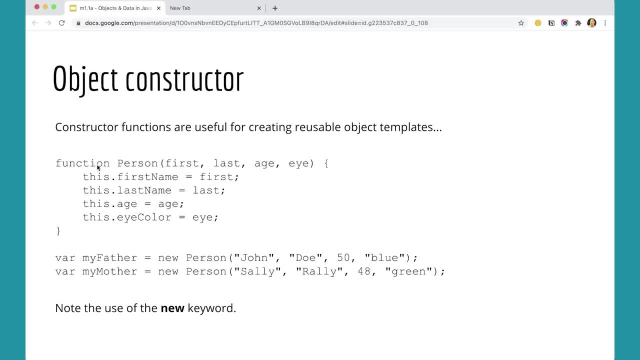 And we're going to pass in some values First, Last Age And eye color, And you could have other values if you wanted to as well: Height, Weight, Hair color, I don't know Whatever other things you want to use. 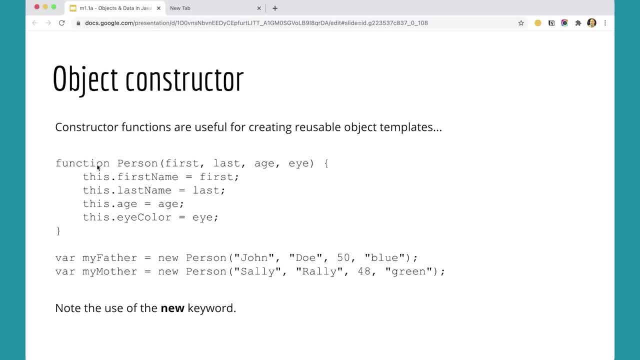 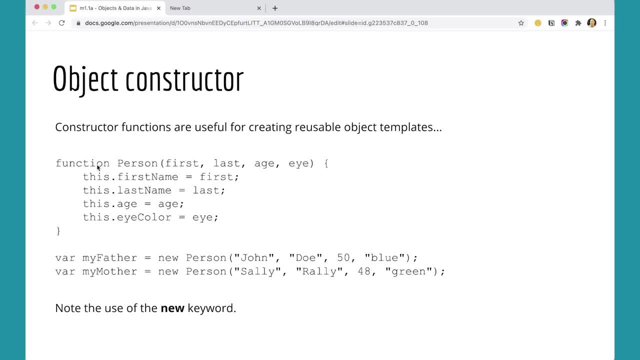 And Notice we're using the, This keyword. This First name Creates a first name Property On person And it's going to be assigned, Whatever gets passed in, As the value For first When the, When the object is. 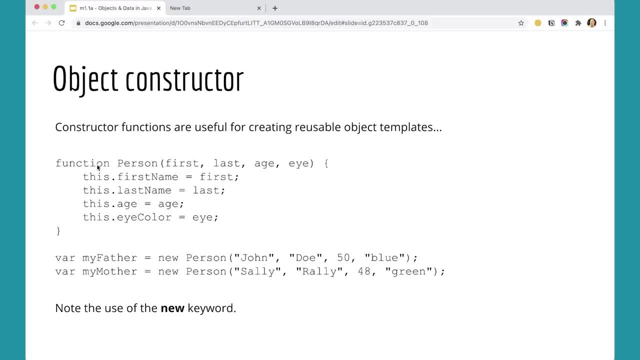 Instantiated, And the same thing for last name And age And eye color. So let's give this a try To see how it works, And I really recommend Typing this out, Because We're starting to have Seen. 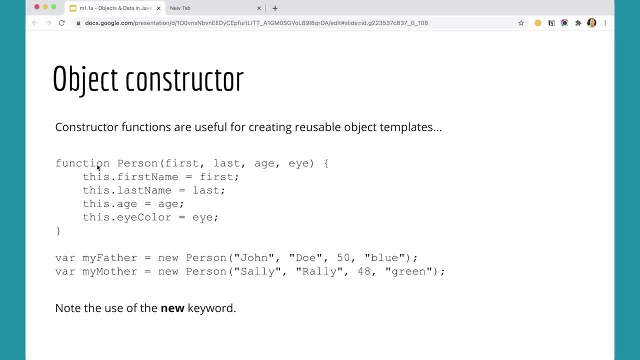 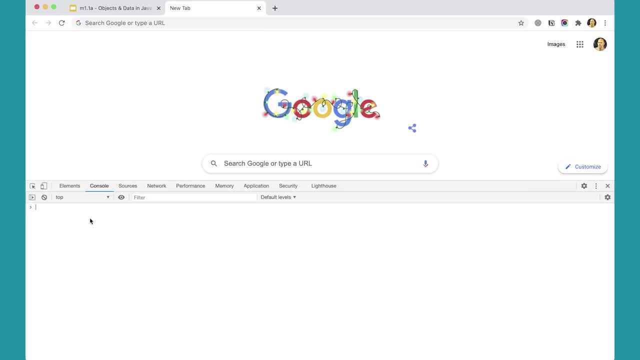 A number of different ways Of using objects Now, And if you're not typing them, You're not going to get comfortable With them Or remember them. So I'm going to go over here, To my tab Here, And I'm just going to paste it in. 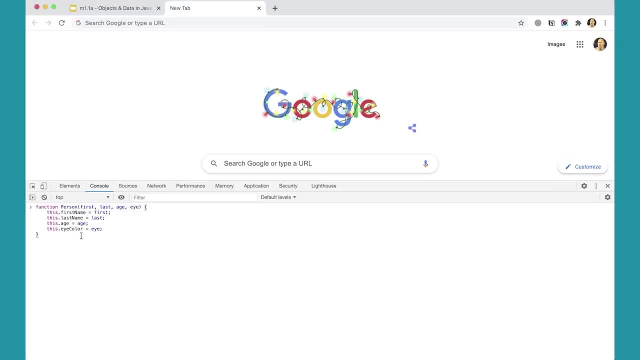 But You should definitely type it. Type this whole thing out Here, And Once I put this in here And press Return Or enter On my keyboard, I can then make A A copy of this person. Use this as a template. 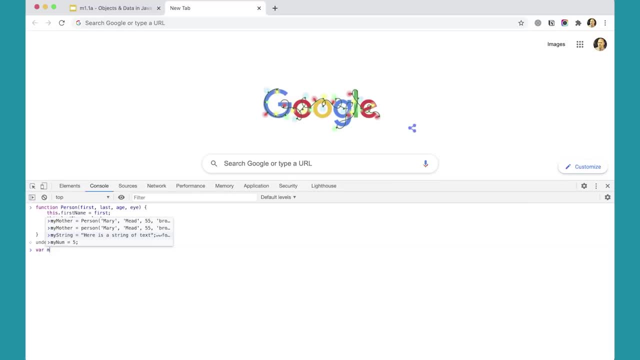 So I could say something like Var, My Mother, And I can assign it Using The new Keyword, New Person Notice with the capital P, And then In here I'm going to put in: 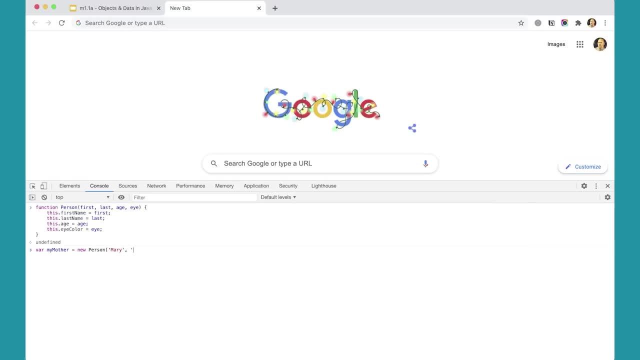 First name: Mary Comma Mead Comma, Age 60. Maybe, I don't know Whatever you want to put. And then Eye color, I don't know- Brown. So now I have A copy of this object. 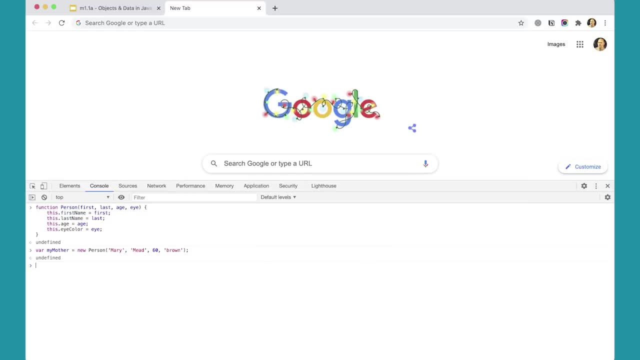 In My mother And I can access its values By typing My mother Dot First name. It's that second one there. Oh no, We had first name With a capital And that gets me married. So There we go. 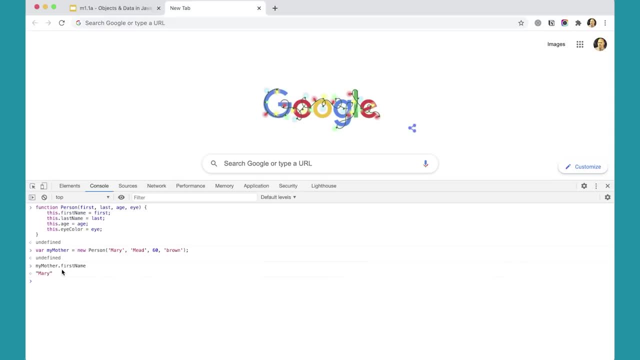 We can actually access these values For this object here, And I can make another object Bar. My father Equals New Person: George Mead, 85. Green. I don't know Something like that. And now, 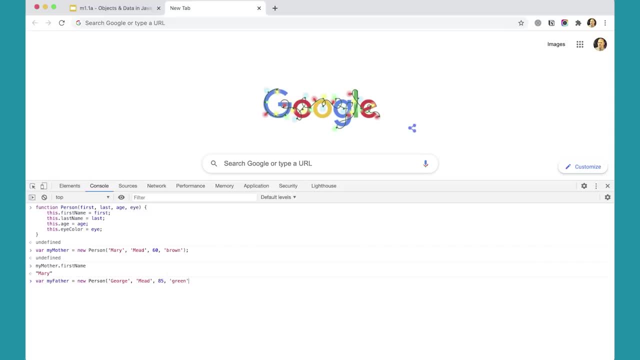 I can access My father, My father Dot Last name, And you'll see That I get Mead. So I can use. I can Use this Constructor Function To create Objects That are: 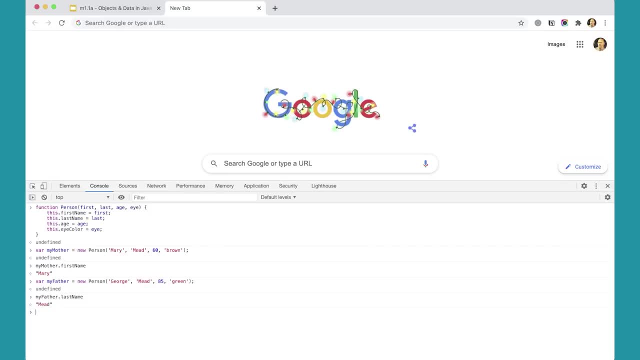 In My Mother, So I can Use This To create Objects That are Reusable Objects And can have Different Values For each Time You instantiate A new Object From that. 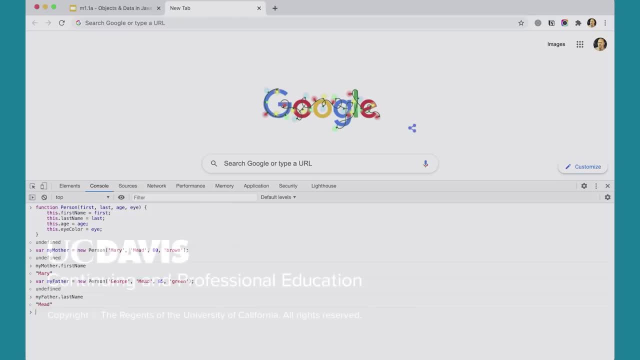 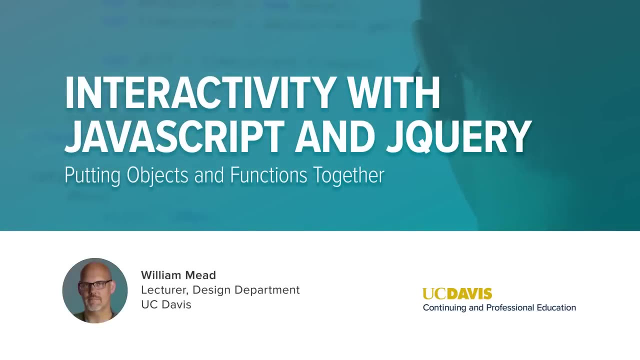 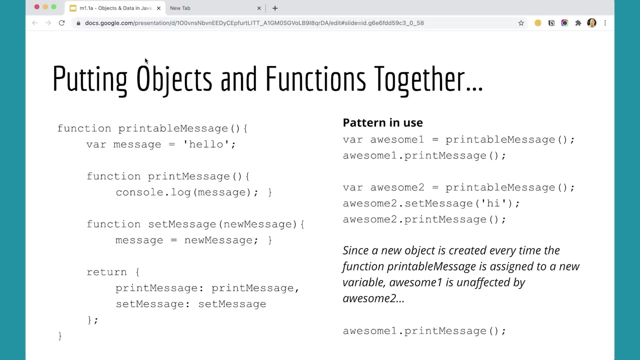 Constructor Function, And this Is a very Powerful Pattern That you'll See Frequently In More Sophisticated, More Complex JavaScript Programming, And we're Not Going To Do. 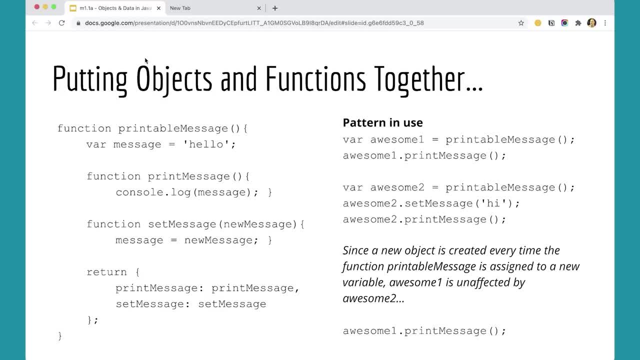 Anything In This Course That's Going To Really Make Use Of A Pattern Like This, But I Want To Show It To You As And. 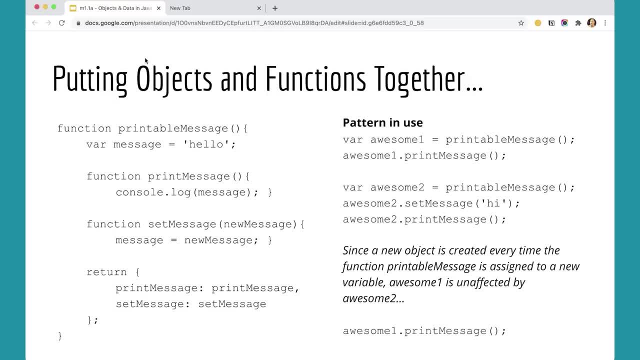 Then I Have Another Function In Here, Called Print Message, Which All It Does Is Print Out That Value. That's, Inside The Message, Variable. But 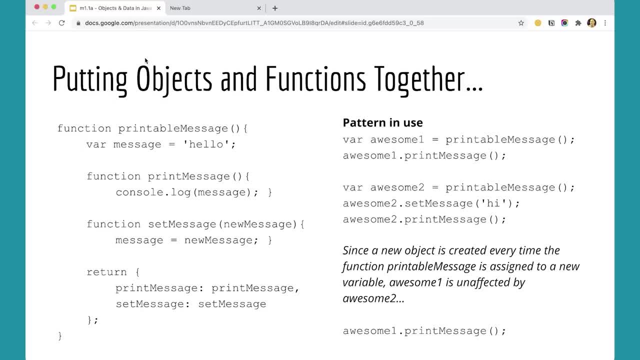 I Have Another. The Object That It Returns Has Two Members As Print Message. The Function Print Message Is Returned And The Function Set Message Is. 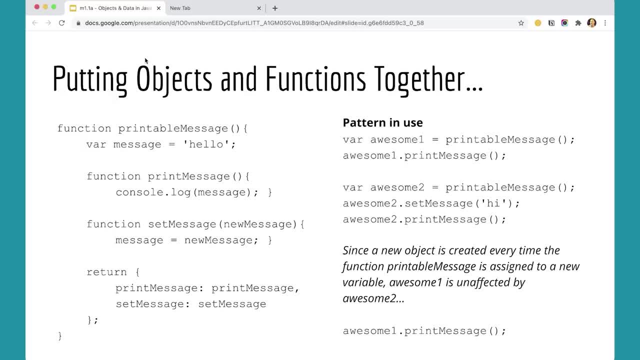 Returned, And So We Can Use Any Function In JavaScript As A Closure. However We've We've Talked About Scoping Closures, And This Is 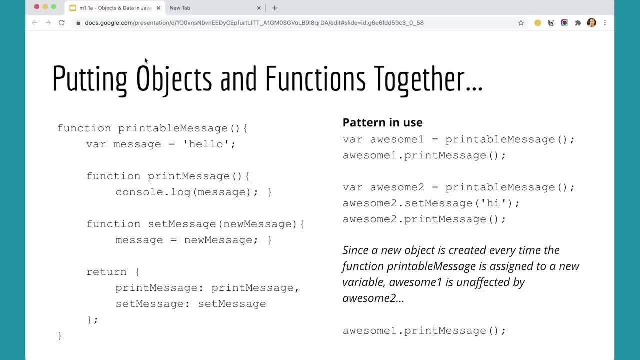 Kind Of A Really Good Example Of The Power Of A Closure, And Again I Strongly Recommend That You Actually Print This Out, Type This: 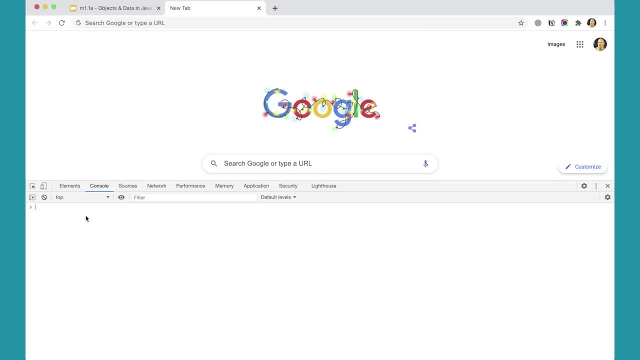 Out And Put It Into. You Could Either Put It Into An HTML File And Send Printable Message With Parentheses There, And I Can Do. 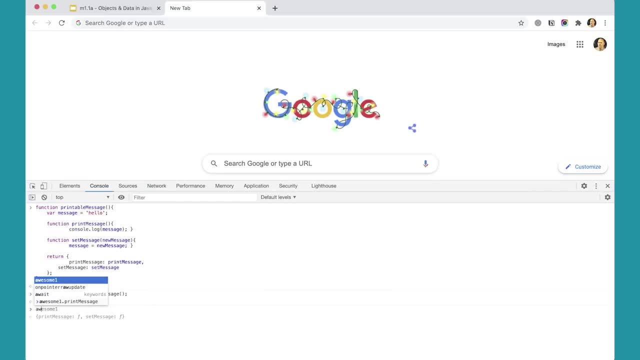 Awesome. One Dot Print Message Parentheses And Run That Function In There And Give Me Hello. But I Could Also Make Another Variable Bar- Awesome. 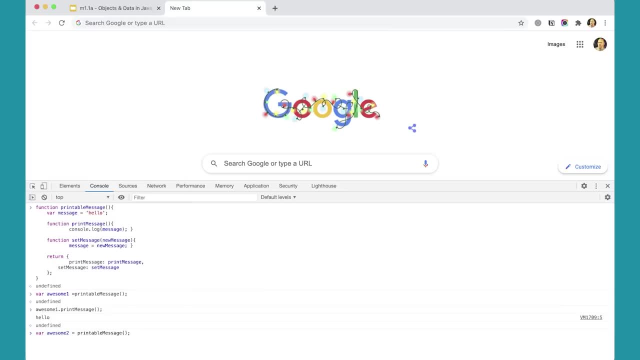 To And Assign It Also That Same Function: Printable Message. Printable Message- Dot Set Message And I'm Going To Put In A New Message Greetings. 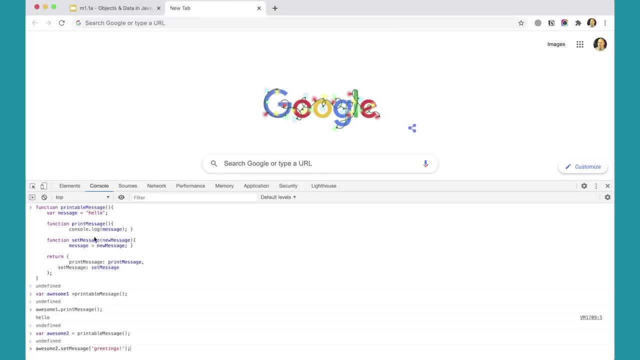 Like So And What That Will Do Is It'll Go In, It'll Run This Function And If I Do, Awesome To Dot Print Message I. 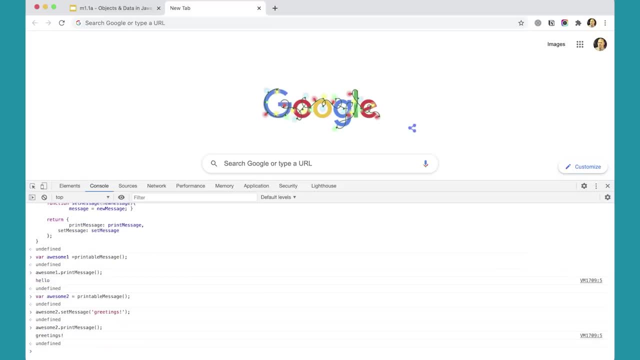 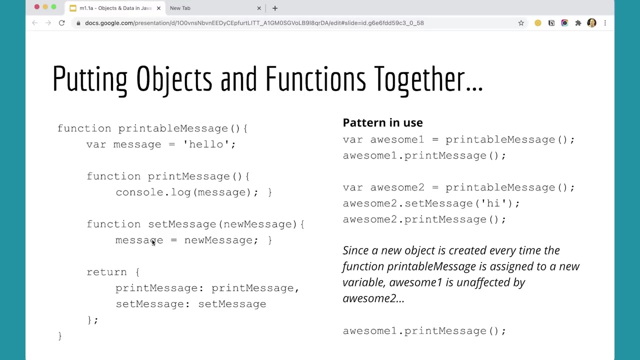 Get Greetings. However, Again, If I Do Awesome One Dot Print Message, I Still Get Message In A New Message. It's Really Interesting That I. 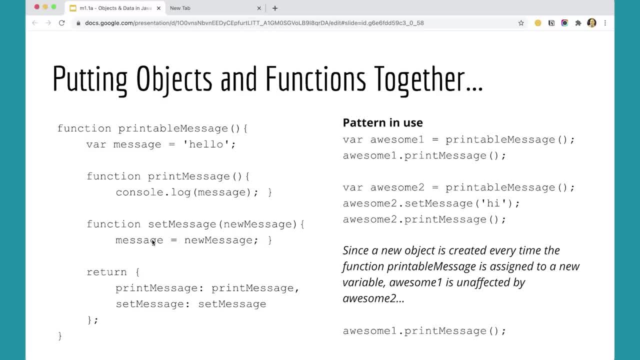 Can Actually Use This Pattern Here To Set Different Values And Then Access Those Values In Different Ways Through And You This Opportunity To Create Things. 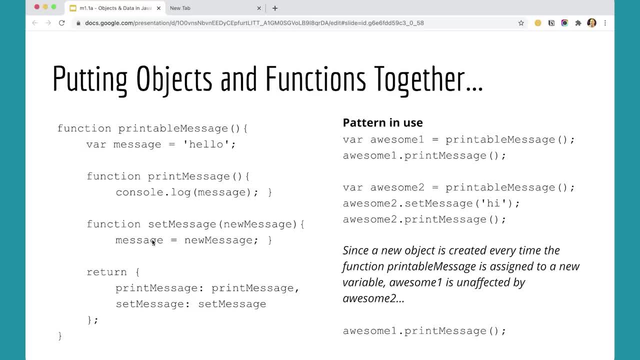 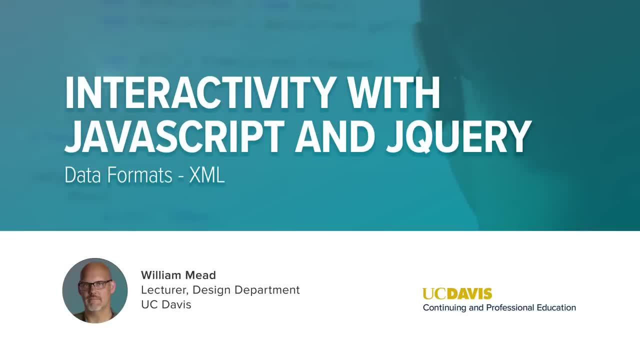 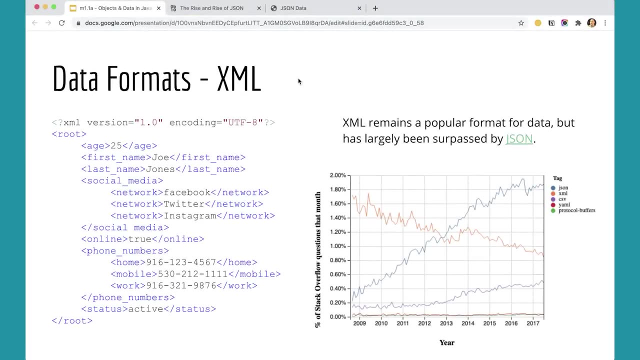 That Are Reusable, Reusable Modules- And That's A Key Thing In Any Programming Language- Is To Be Able To Do That. The Data Format. 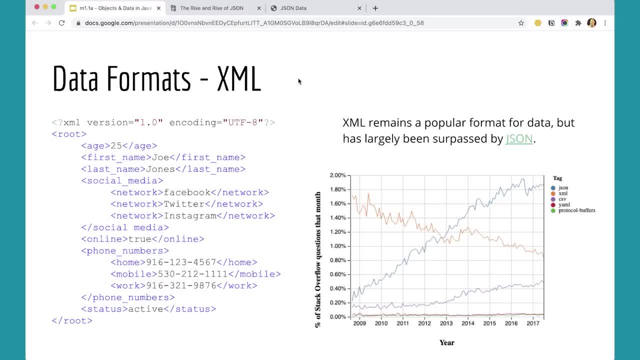 Called XML And, If You Look At It, Should Look Fairly Familiar, In The Sense That We Have Data That Has Been Described Using 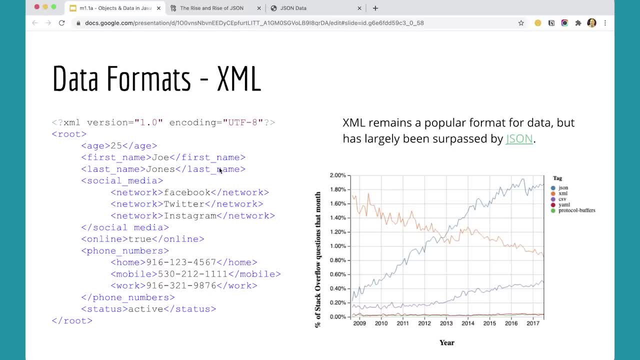 Tags And The Data, So You Can Actually Create Whatever Tags You Want. That Will Help Describe Your Data, And XML Was And Is A Very 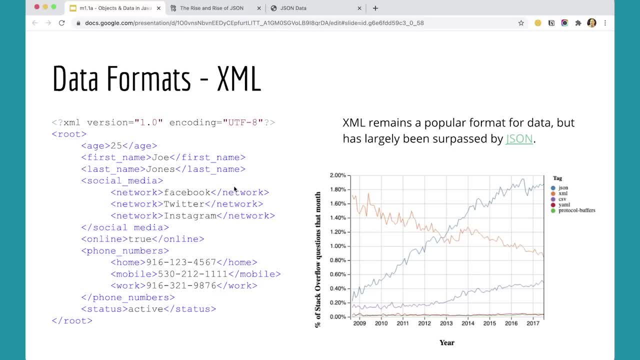 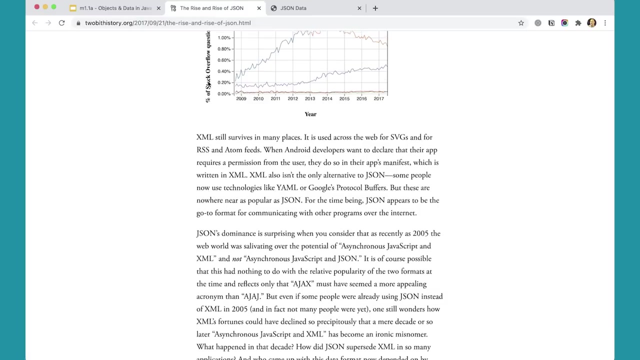 Popular Format Has Been For A By Another Data Format Called JSON, Which Stands For JavaScript Object Notation, And Over Here We Have A Graph. 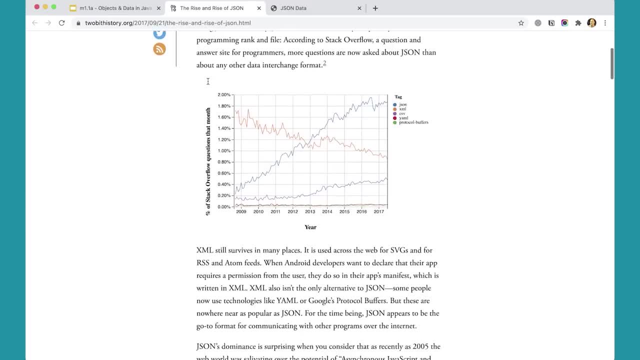 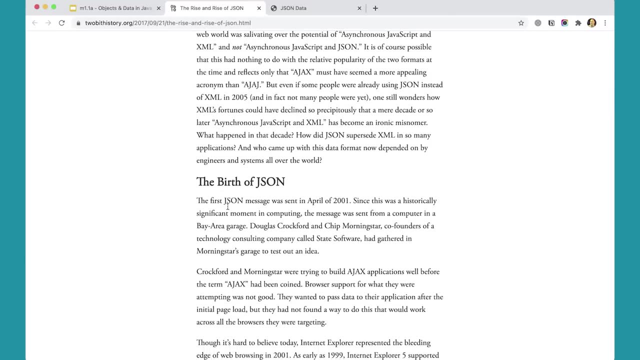 Here About, About Sort Of The Popularity Of These. And You'll Also Notice This Name: Douglas Crockford Was Involved With The Invention Of 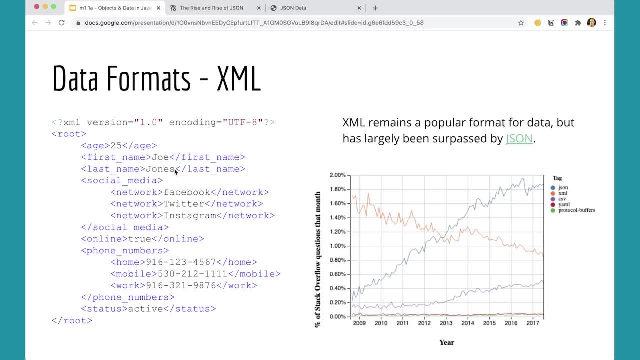 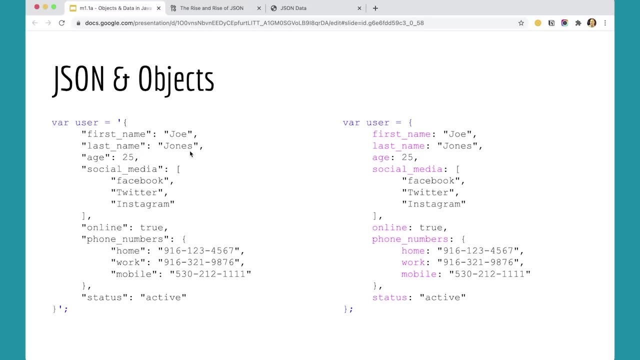 This Data Format, JSON. We've Talked About Him Before, So XML Is A Valuable Format For Data, JSON And Objects. Now On The Left: 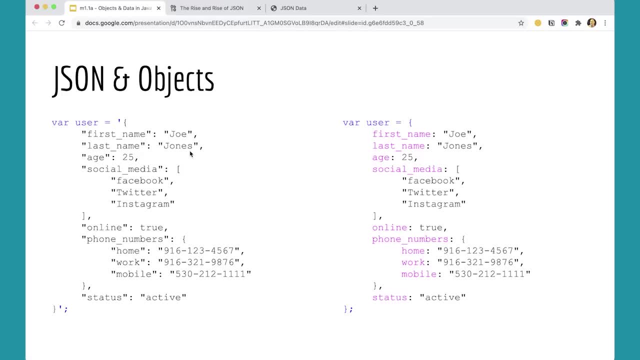 You'll See Something That Is JSON Formatted. JSON Formatted Strings. This Is Data In JSON Format. Again, JavaScript Object Notation And On The JSON. 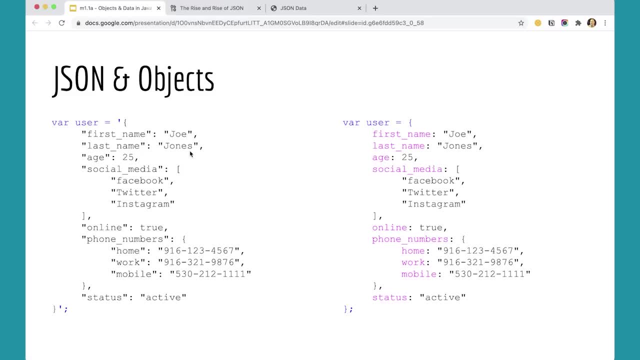 The Whole Thing Is A String, So You'll Notice That There's A Quote Mark Right At The Very Top And A Quote Mark Right At 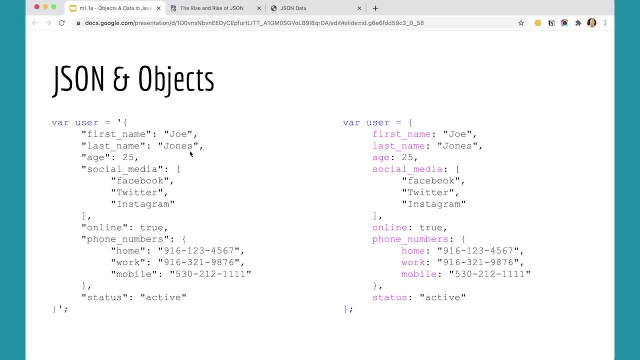 The Bottom Two. But Other Than That, They're Very Similar To Each Other In The Way They Look, In The Way They Act. So We 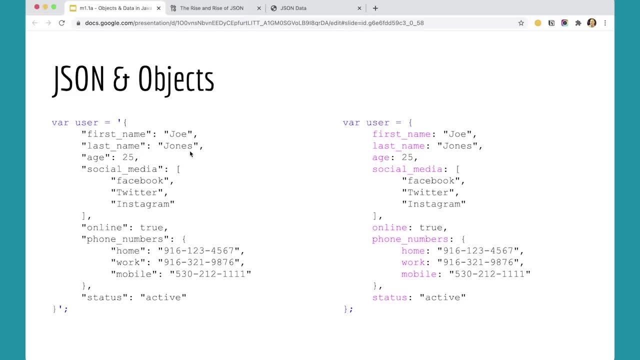 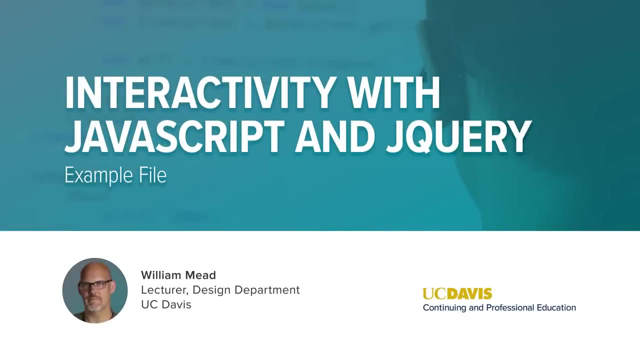 Are Familiar With This Format. Right Then, You're Going To Convert That Data Into An Object That You Can Manipulate And Use Within Your 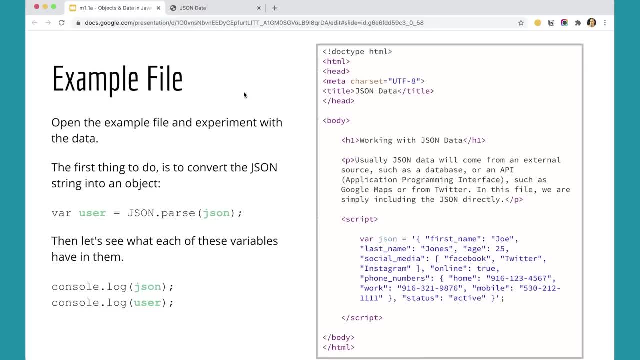 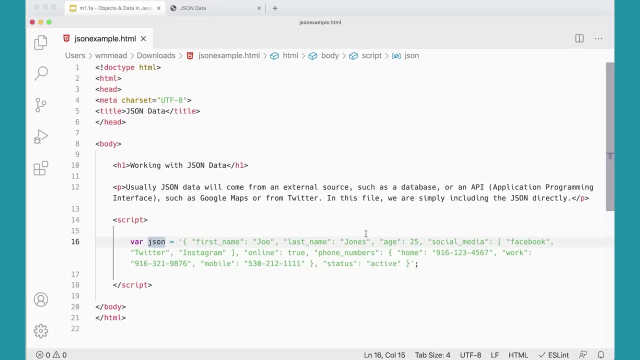 JavaScript Program. With This Lesson There Is A Example File. So With That File With Some JSON Data, So I Have That File Open Over Here. 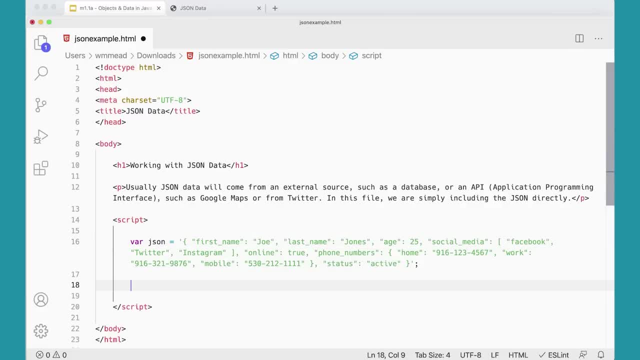 And In It Is Just A Variable Called JSON With A String Of JSON Data, JSON Dot Parse. I Think It Needs To Be Capital Letters. 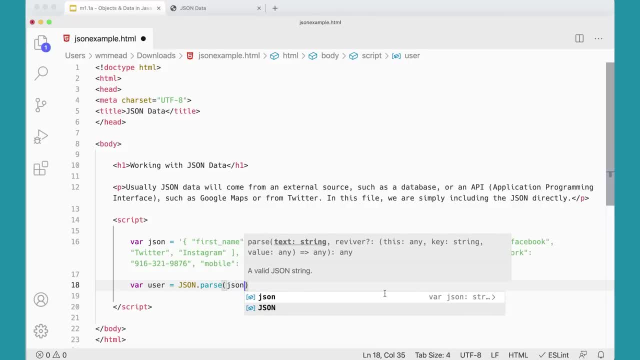 And We Pass In The JSON This Variable Here, Great. So Now Let's See What Happens. We're Going To First, I'm Going To Console. 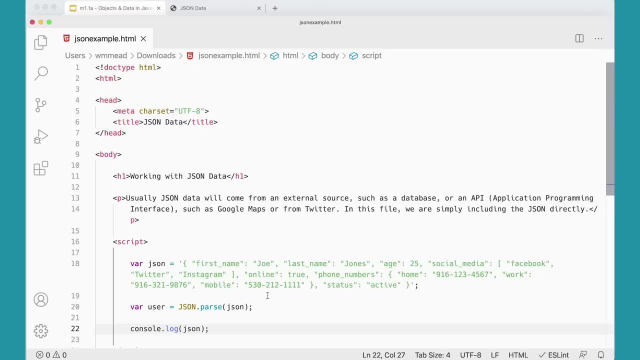 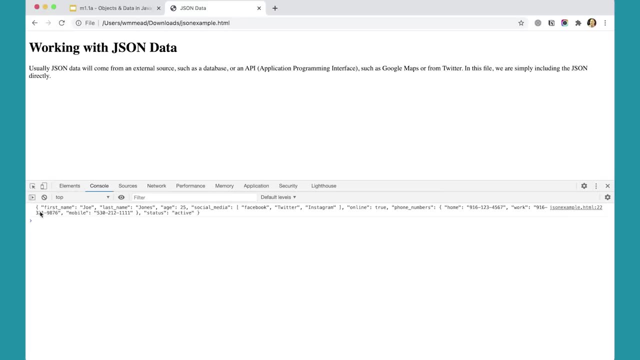 Dot Log. I'm Just Going To Console Log The JSON Variable Up There And That Should Just Give Me Some External Source, Maybe From A. 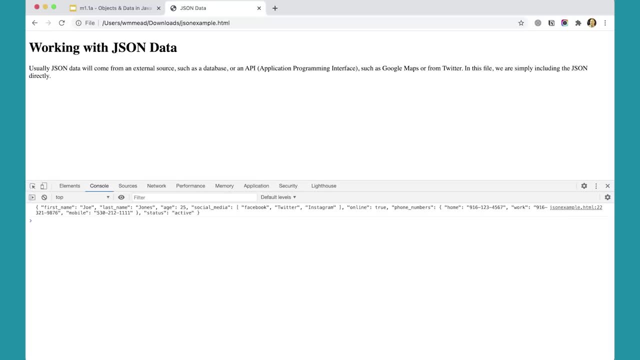 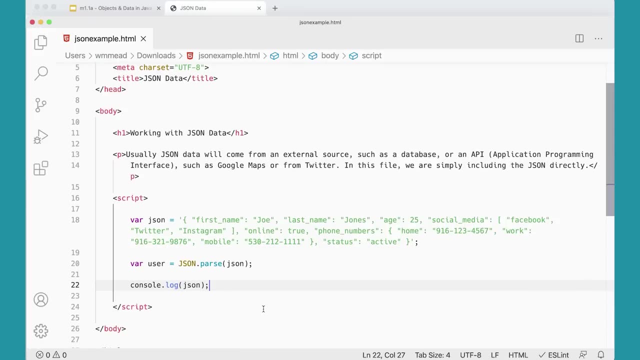 Database Or From Some Third Party API, And We'll Be Talking About The Those Later In This Course, But For Right Now I've Got Some 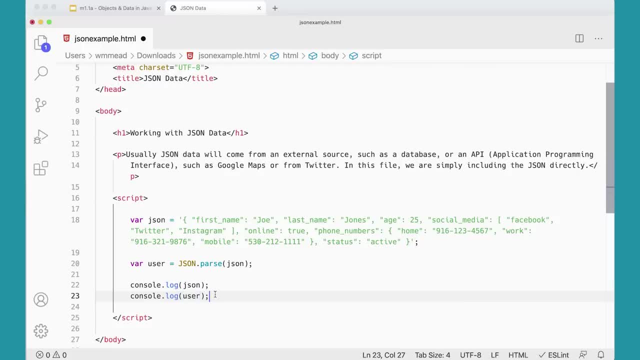 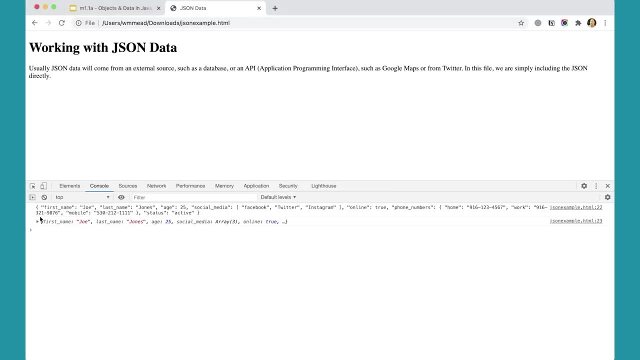 Data. I'm Going To Console Log. I'm Just Going To Console Data Right Now. I'm Going To Console. Right Now, I'm Going To Console. 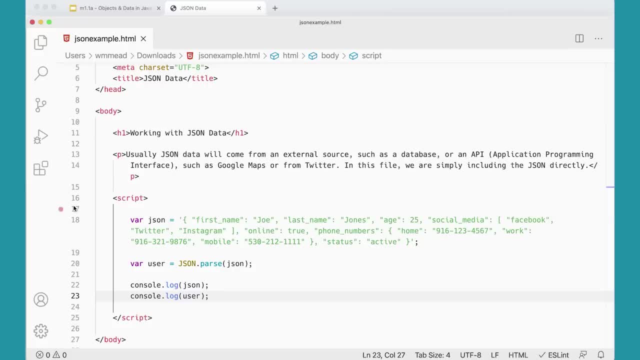 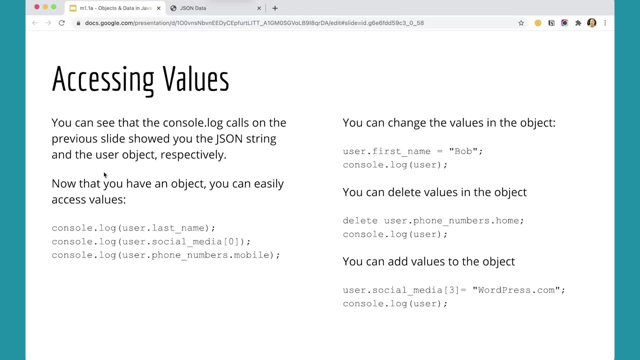 Right Now I'm Going To Console This Parse Method Here. Takes That JSON And JSON Parse Will. Take That JSON And Parse It And Stick. 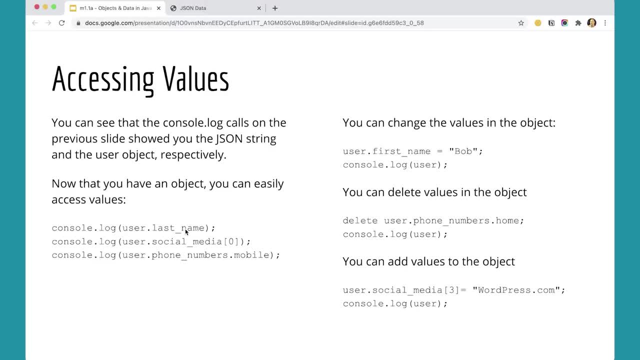 It Into User. So Now It's An Object. We Can Change The Values Of An Object. We Talked About This A Little Bit Before, But 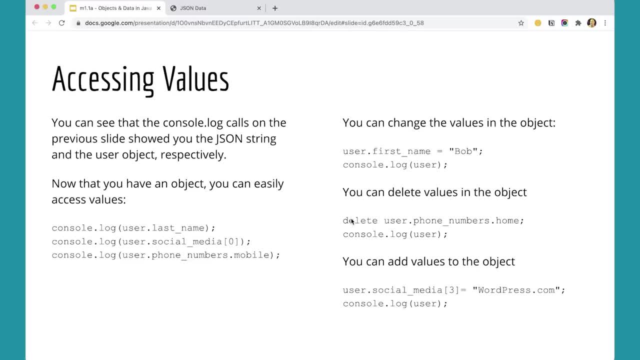 I Can Just Assign A New Value And If I Console Log Out From My Object, From My Data, And If I Console Log Out User. 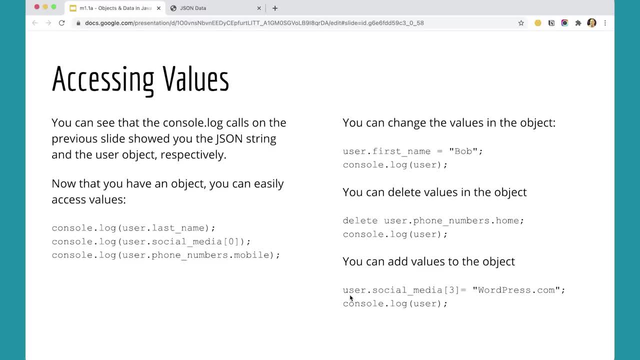 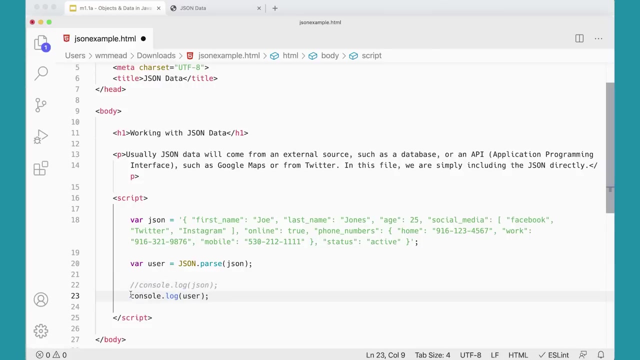 You'll See That It's Gone. I Could Add Objects, Add Values To The Objects, So These Things Out. If You Go Over Here And Just 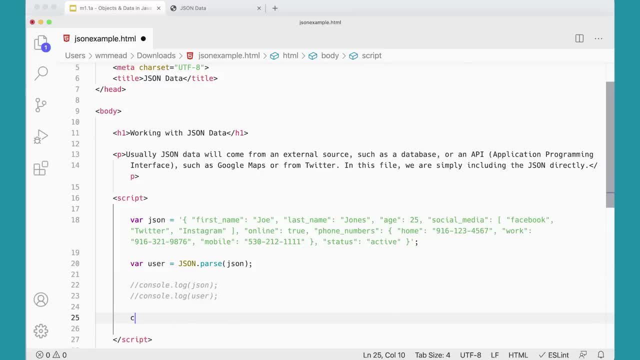 Add Some Calls To The Console Log. You Can Comment These Out If You Don't Want To Actually See. It Should Work. Come Back Here. 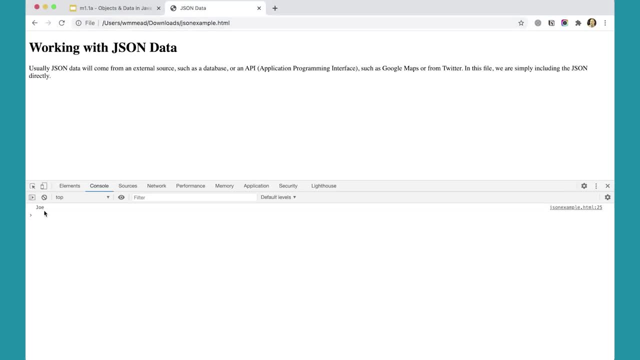 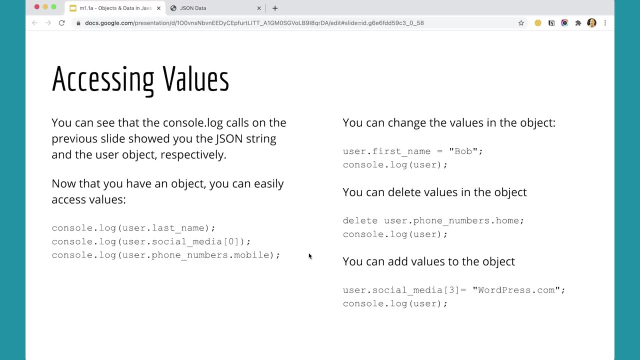 And Refresh This. I'm Getting Joe So You Can Go Through And Try Some Of These Different Pieces Here. I Strongly Recommend That, You Know. 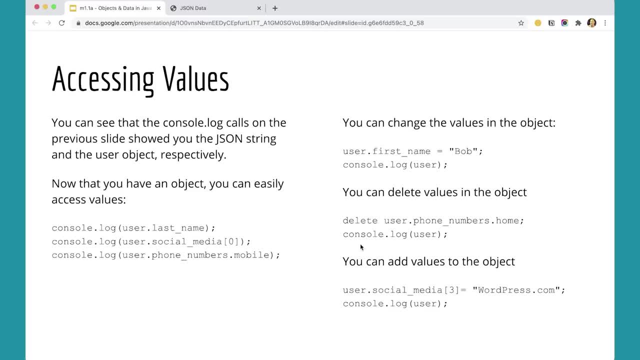 One Thing Students Tell Me When I'm Teaching JavaScript Is I Didn't Spend Enough Time On Objects, And Really The Truth Is They Didn't. 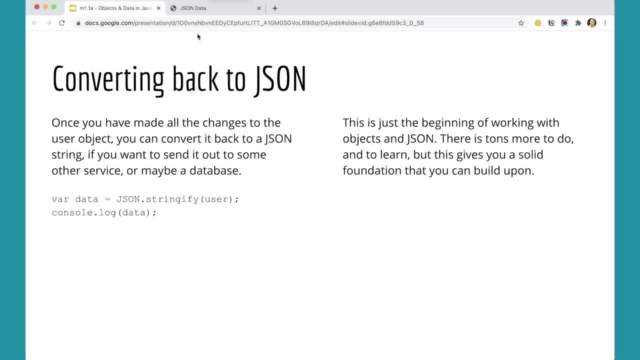 Spend Enough Time On An Object And Converted Back Into Json Or Converted Into Json, And You Can Do That By Simply Doing Using The Stringify. 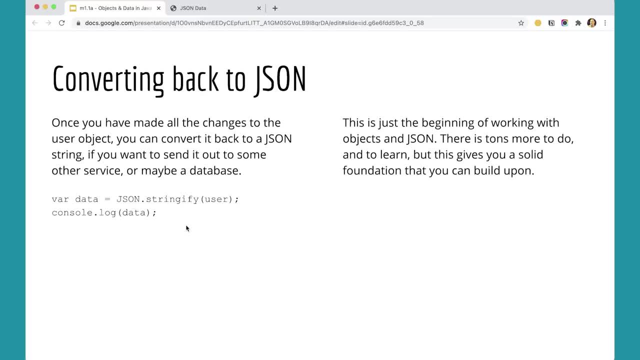 Method With Our Using The Json Object. We Want To Do That. You Suppose You Want To Create An Api And You Want People To Access. 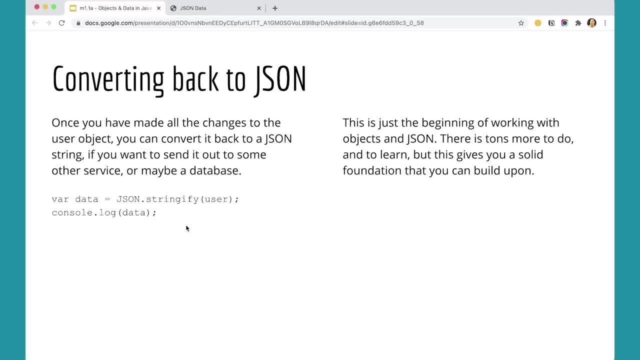 Your Data. You Might Need To Take Some Data That's Very Important To Build A Object And Turn It Into A Json String Using The 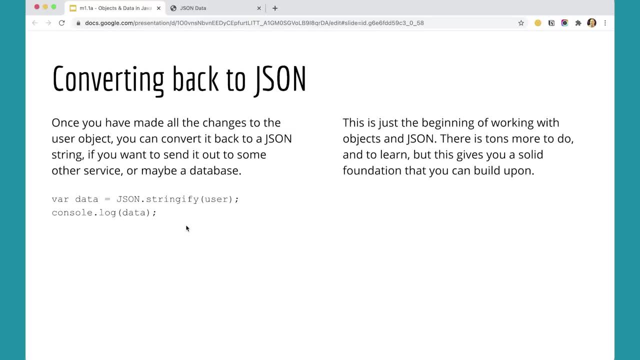 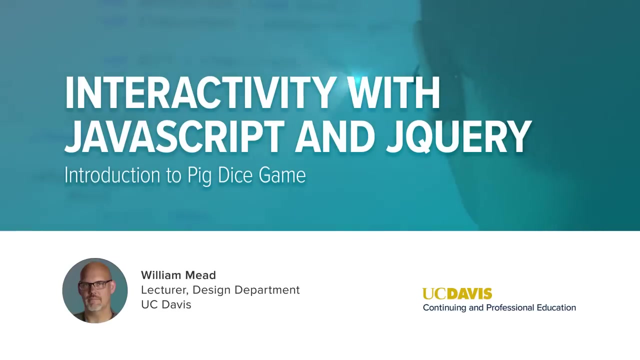 Stringify Method So You Could Go Back And Forth Between Json And An Object To Build An Object In This Course. But I Want To. 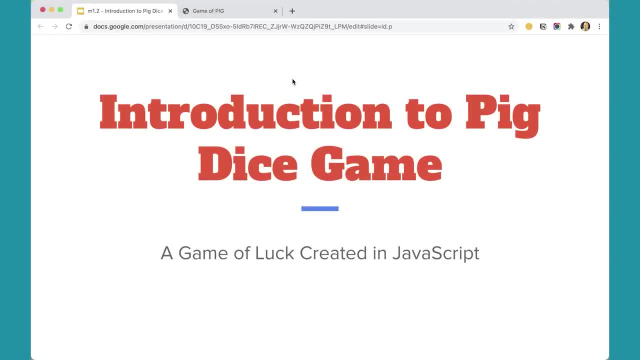 Introduce You To The Topics. Introduction To Pig Dice Game. This Is A Game Of Luck. Created That Lesson I'm Hoping You Can Make. 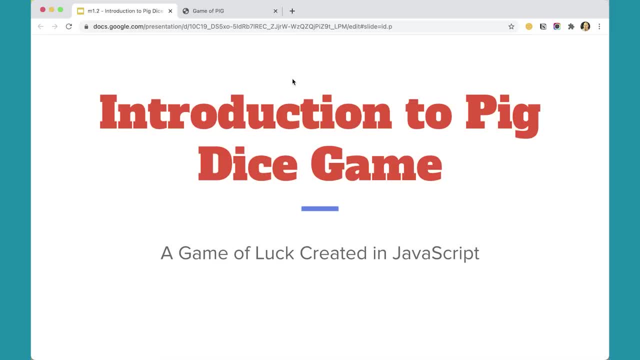 Some Of Your Own Variations Of This Game And Make It More Interesting My Variation Of This Game. So We've Been Working In Kind Of. 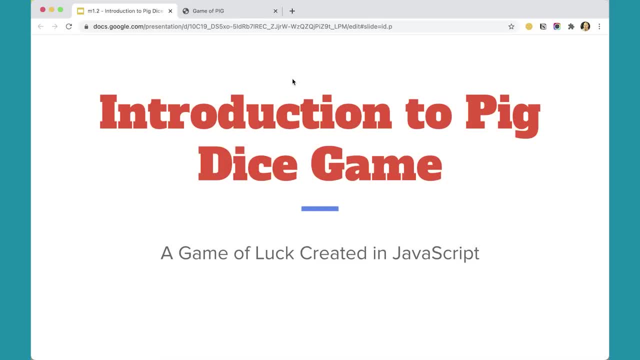 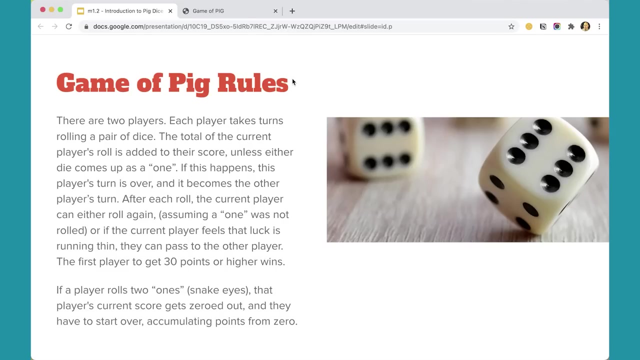 A Very Limited Scope Now, As We Get Into Working With Data, With JavaScript, And We Start Thinking About Creating More Sophisticated Applications, Our Scripts. 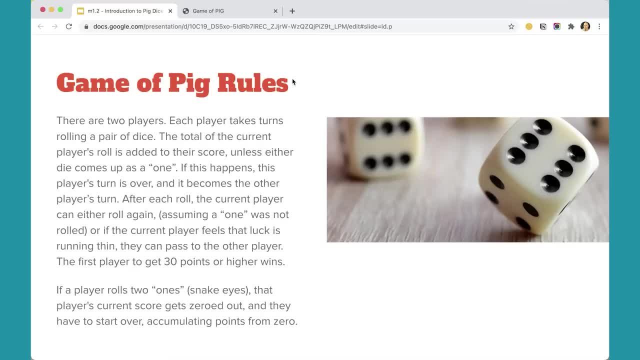 Are Going Back To The Game Of. Our Version Of The Game Is That There Are Two Players And Each Player Takes Turns Rolling A Pair. 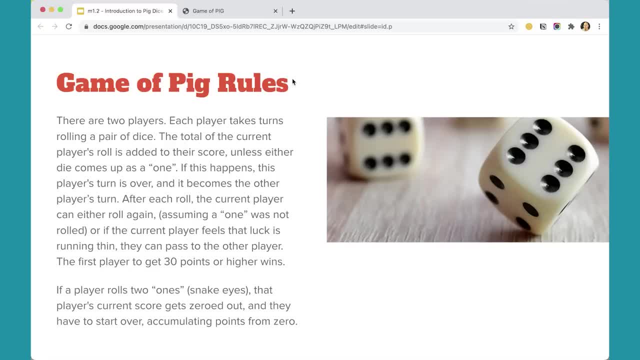 Of Dice, The Total Of Dice, Roll Again With The Hope Of Adding To Their Score And, Assuming A One Was Not Rolled, They Can Roll. 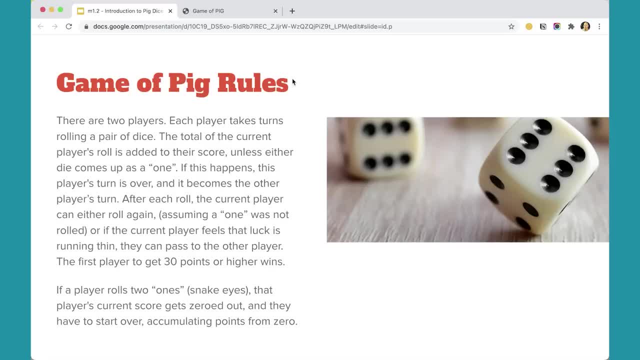 Again, Or If The Player Feels That Luck Scratch Accumulating Points From Zero. So Those Are The Rules That We're Going To Play With. 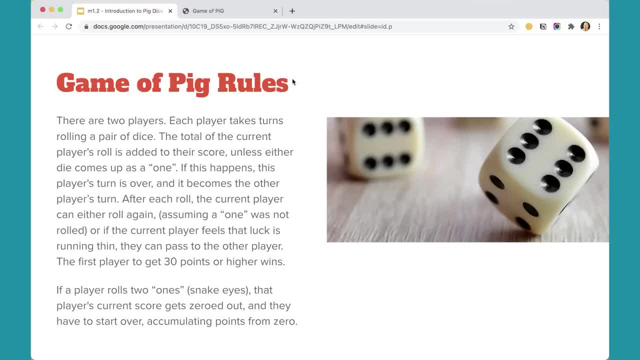 And The First Thing To Do Is To Really Think About These Rules, Programmers, Or In These Lessons Generally, I Present Sort Of How To. 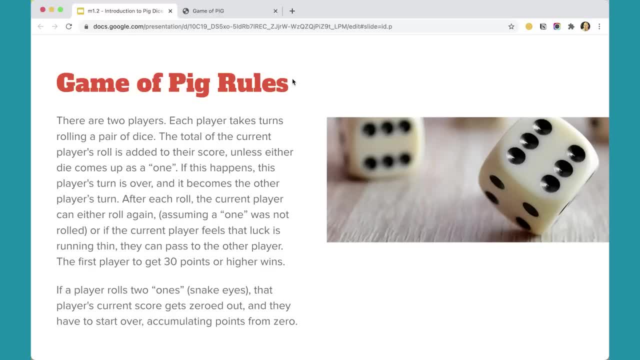 Make These Types Of Things In A Logical, Linear Fashion, But It's Really Important To Understand That That's Not How The Game Was Created In. 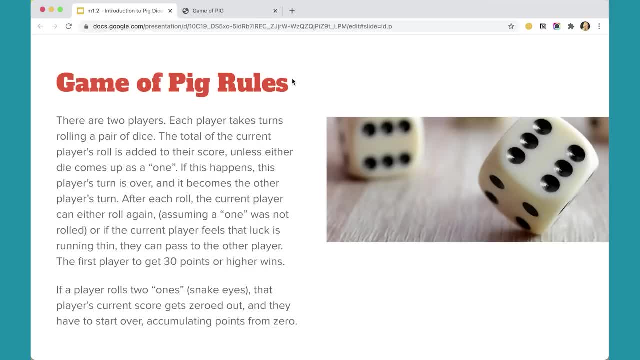 A Logical, Linear Way. So What We Need To Do Here, What I Really Want You To Get Out Of This, That's Not How I. 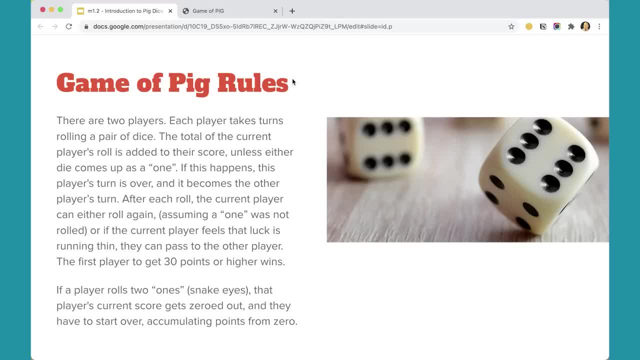 Created It And To Really Sort Of Think About The Process Needed In Order To Go About Creating Something More Complex Like This. And It's 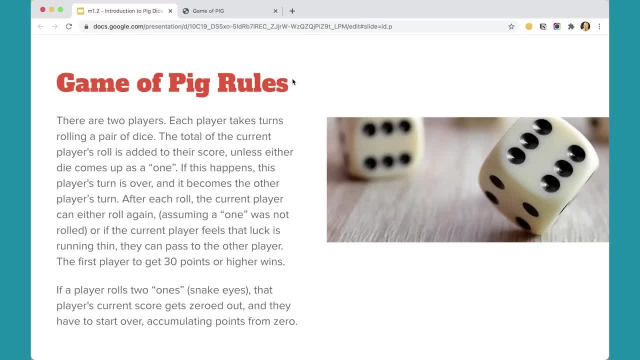 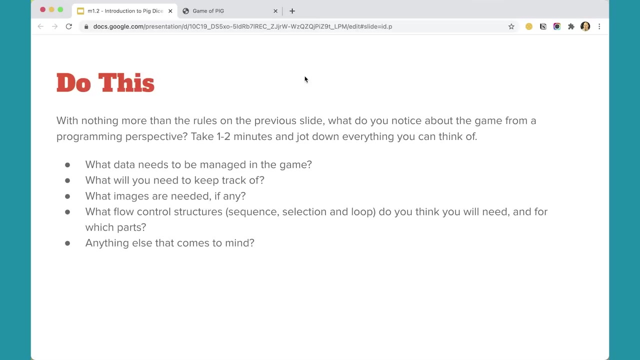 So That's Going To Be The Process We Go Through Here, And I Really Strongly Recommend That You Do These Steps And That You Really 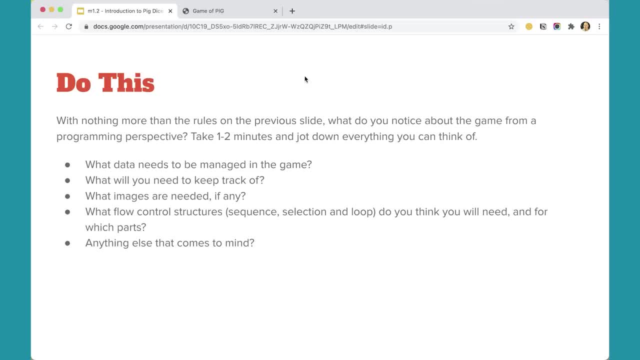 Think About This As From A Programming Perspective. Get A Piece Of Paper, Get A Pen, Pause This Video Or Stop The Video And Jot. 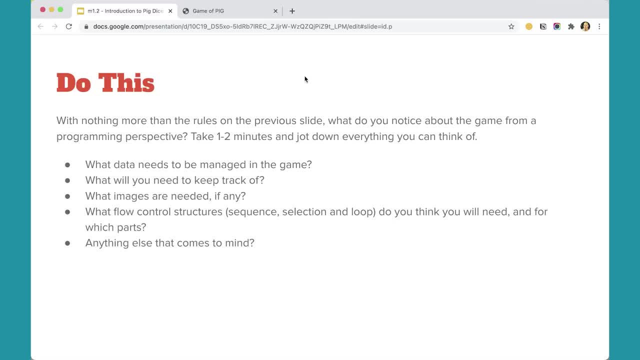 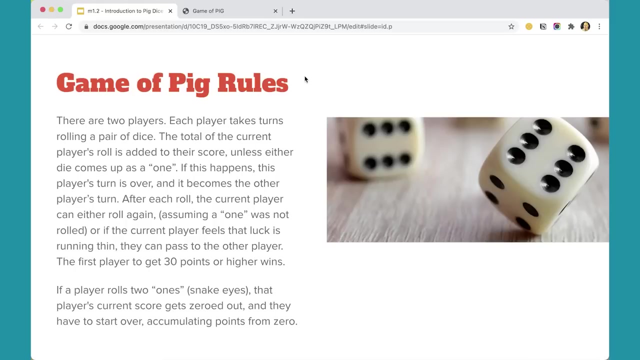 Down Everything You Can Think Of What Data Needs And For Which Parts. What Else Comes To Mind, Just With Nothing Other Than The Rules Sit. 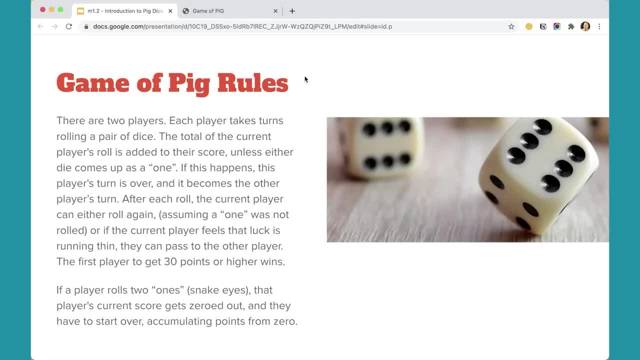 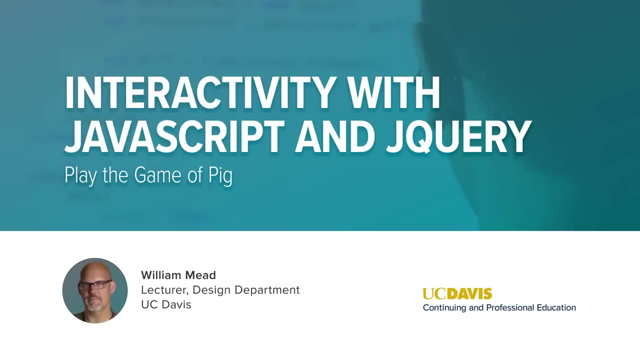 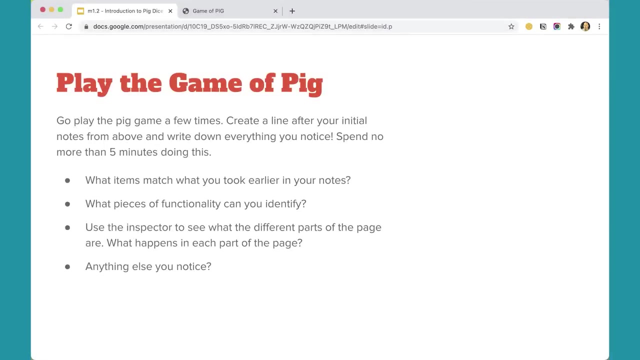 Down And Take A Few Minutes To Think About This And To Think About The Rules. Okay, Now, Hopefully You've Taken A Few Minutes And 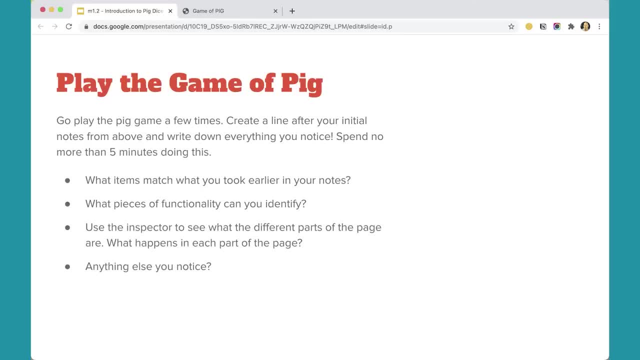 Jotted Down Some Notes Just Based On The Rules. If You Are Creating A Game From Exists, So We Can Actually Reverse, Engineer It A. 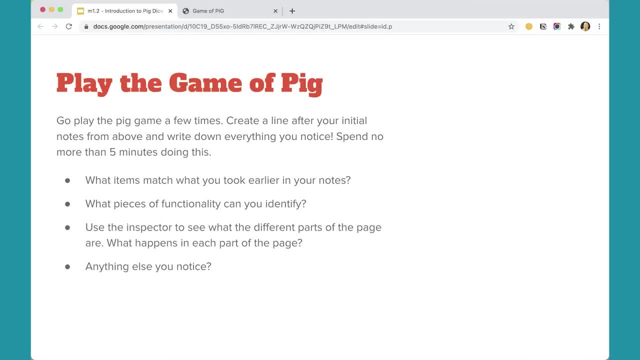 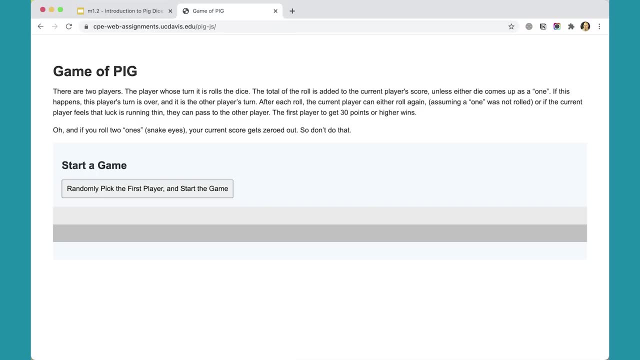 Little Bit. We Can Actually Go Play The Game And Take Further Notes Based On What We Observe While Playing. That I Have And I 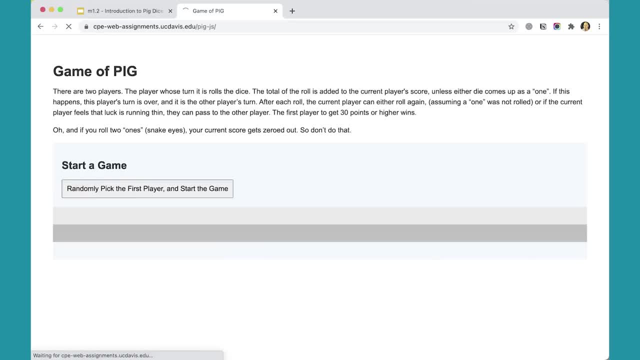 Recommend That You Do This A Few Times. Play The Game Player. See What Happens When You Click The Different Buttons. What Happens If It? 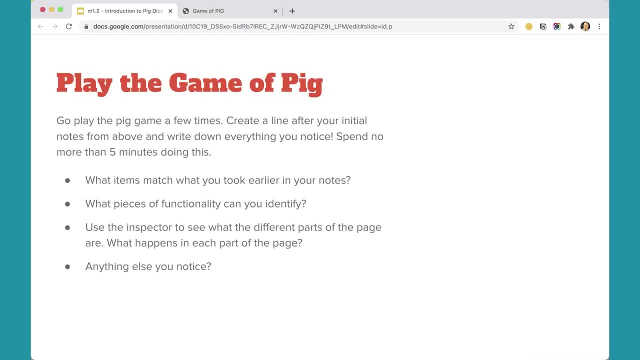 Works, So Play The Game A Few Times. Spend Maybe Five Minutes Playing The Game And Write Down. Spend Five Minutes Writing Down Some Items That. 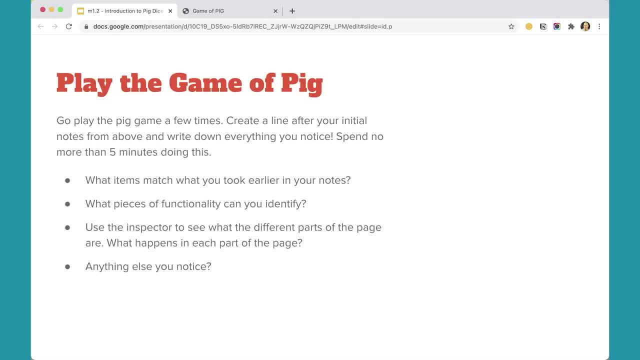 You Might Match What Is Going On Here. There Is A Button. What Can You Observe? There Is A Button. When You Click It, What? 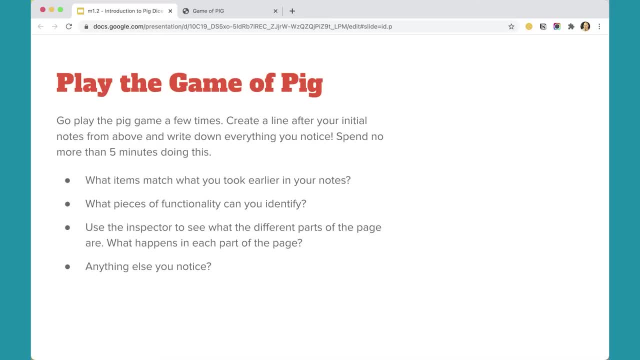 Happens. How Does That Happen? Use That Inspector To Get A News. Is How To Get A New Question. Where To Start If You Don't? 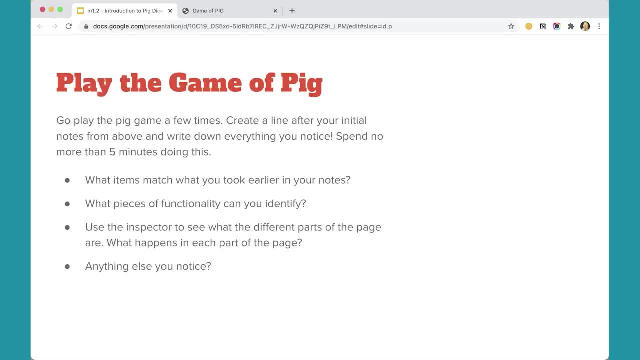 Know Where To Begin. So, Really, This Process Is To Help You With steps as you move forward through the challenges to build something a little bit more complex, And now we're at a point where we're going to make a more complex script that we really need. 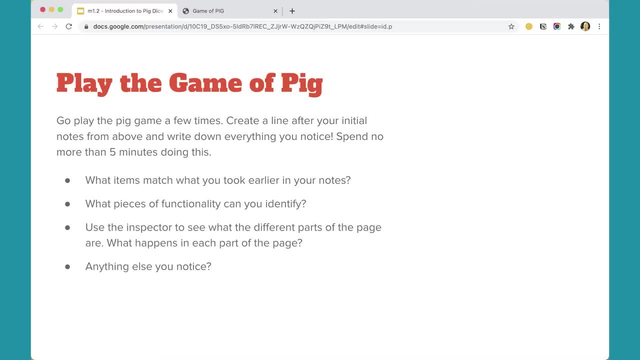 to think about. what are our strategies for doing that? Okay, so take these five minutes and go through and write down whatever notes you can think of. that match what you thought from the previous. from just looking at the rules, Does it match? Are there things that are different than? 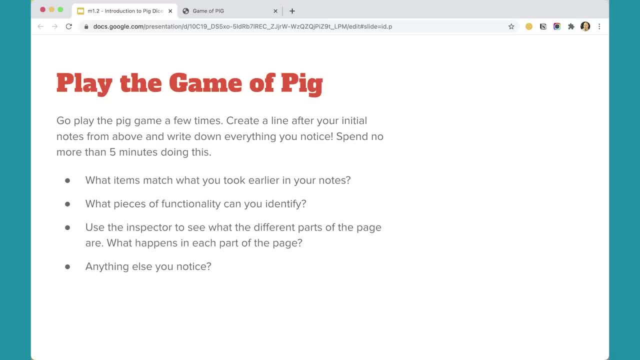 you thought: Are there things that you're noticing that you didn't notice before, since you have the advantage of having a existing version to deconstruct, What do you notice there? Pause the video and do this before going on to the next part of the video. 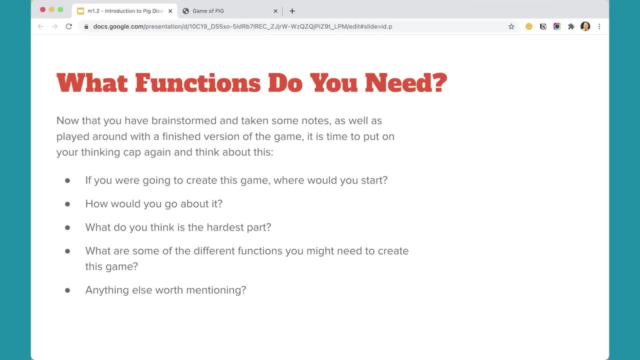 Okay, hopefully you did that and you took some time and wrote down what you needed in your notes. If you did, I'd love to hear from you. If you didn't, I'd love to hear from you. And you went through the game and you played it a few times and you've observed some stuff. 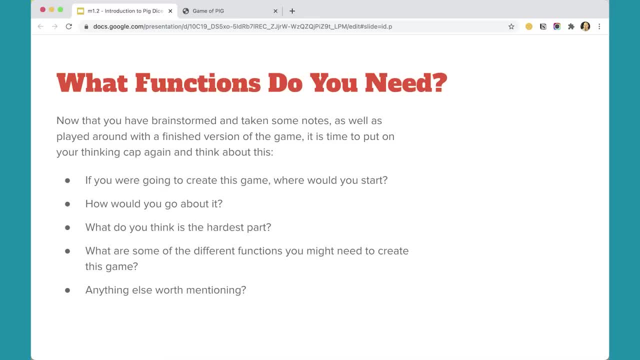 Now it's time to put on your thinking cap and think about how would you go about creating this game using JavaScript. What would you do? You've got some notes to review and you've played around with the game, So where would you start? if you're going to create this game, How would you go about? 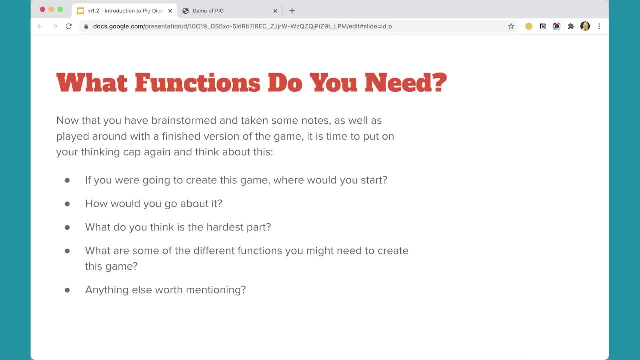 it. What do you think is the hardest part? What are some of the functions you might need to create in the game? What else do you notice? What else is worth mentioning? Really think about this, And what I recommend you do is stop here before going on and take a break from this lesson. Go ride a bicycle. 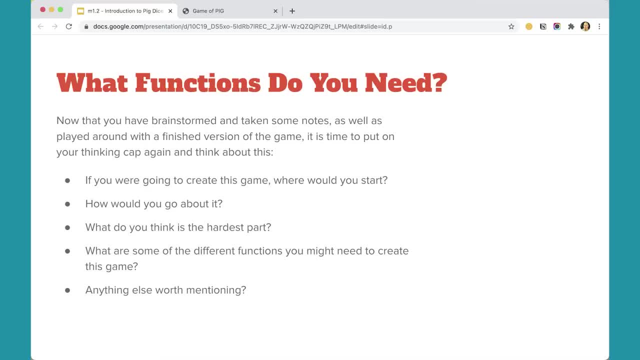 Go take a walk, Go do something else, Something that will allow you to sort of chew on this for a little while and then come back to it in an hour or in a couple of hours, or in the afternoon, or in the morning or tomorrow. 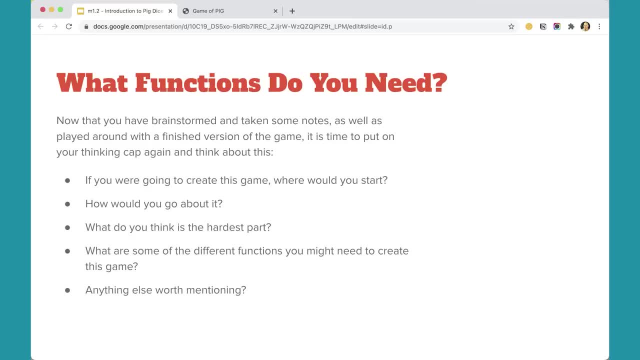 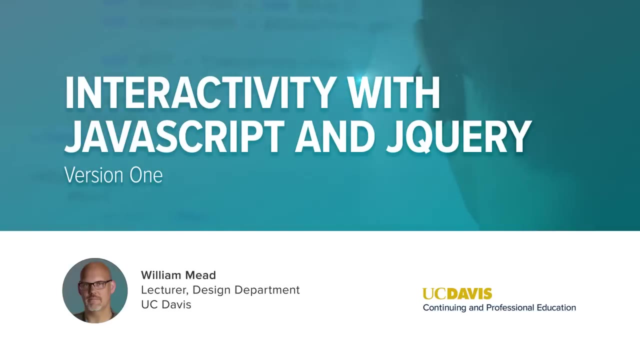 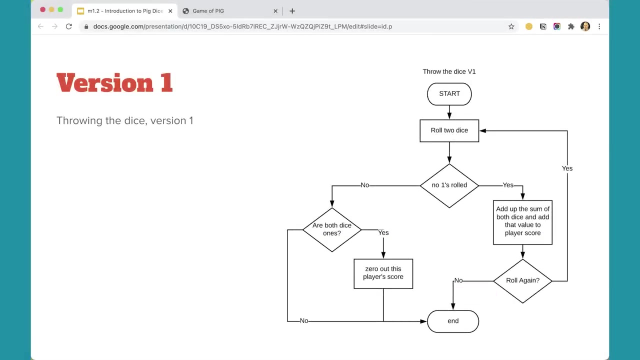 Or something like that. Give it some time, Really percolate on this and think about how you would go about creating this program before going on with this lesson. In this next part of this lesson, I'm going to talk about my thought process for how I go about. 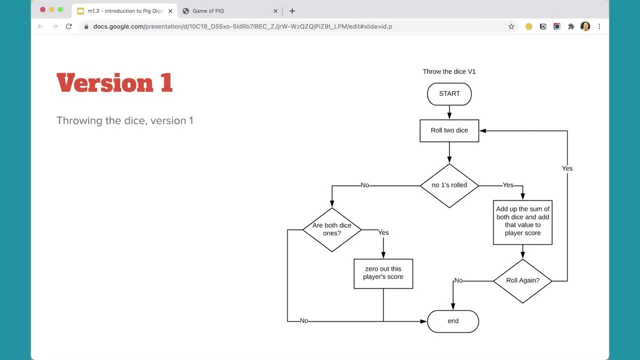 solving these types of problems, And you, your thought process and your problem-solving process may be different from mine, And that's totally okay. I just want to present my thought process because I think it will help with understanding how to go about taking a bigger problem and breaking it down into pieces, And 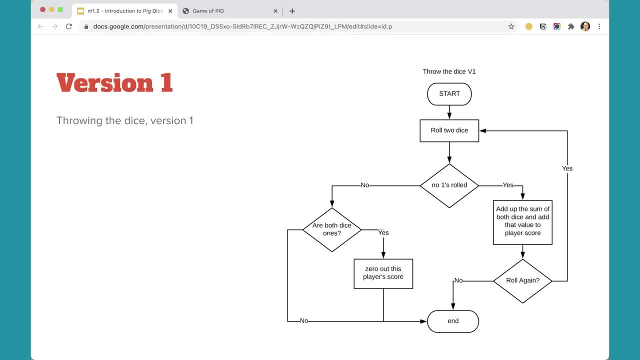 that's something that a lot of people just don't have a lot of practice with. So you have to practice doing this to get good at it. This is not something you just know because you're born knowing how to do it. It's something that you, it's a skill that you develop by practicing it. 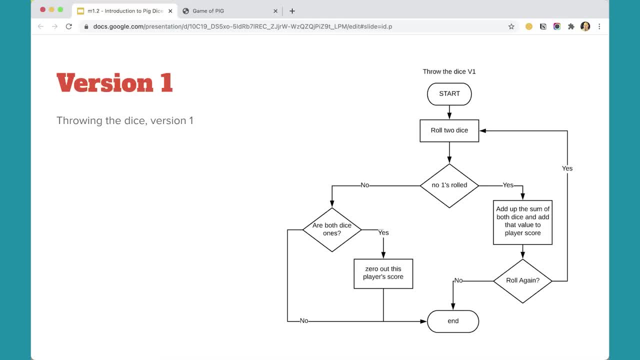 So hopefully you went off and thought about that and thought about how you would go forward And hopefully at the end of this you'll have a sense of how you think about this, differently from how I think about it. So I'm going to show you some, some diagrams here that will walk through. 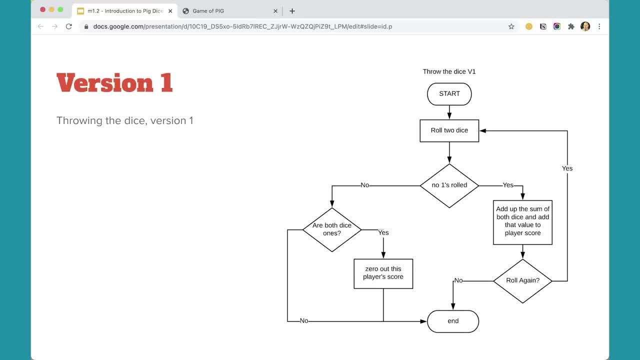 how I think about it, And you can create your own diagrams and you can just draw them on pieces of paper. It's a good idea to do that, to help you sort of think out the steps that you would need in order to do this. The first diagram demonstrates what I think of as the core of this game, and 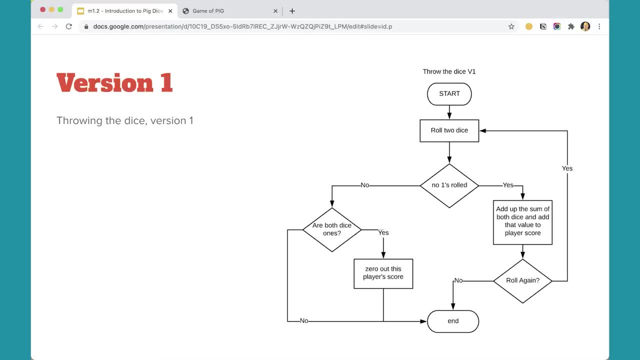 usually for me, when I start a new project, when I start a new challenge, I start with one of two things: Either the hardest part, the thing that I think is going to be the absolute hardest part to solve. solve, Because if I have a project that I want to do and there's a difficult piece to it and I don't, 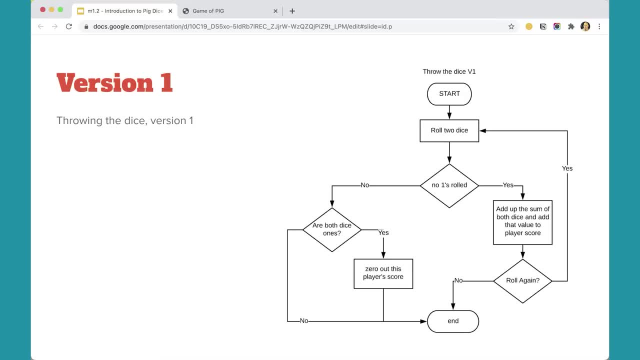 know what that hardest part is going to be. you know, if I don't know if I'm going to be able to solve the hardest part of that, then I want to solve that first before spending time on the easier parts, because I don't want to waste my time. That's one strategy. The second strategy is: 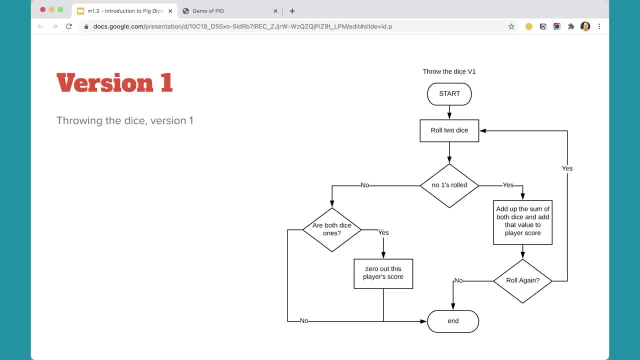 what is the core, What is the absolute, most essential part of the program that you want to create, What is the absolute kernel core of it? And that was my approach with this game. So, when I think about this game, the core action of this game is a roll of the dice. 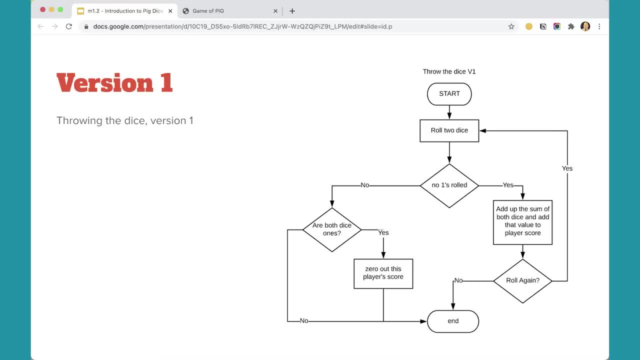 A player rolls the dice and something happens, And then decisions are made in the game based on what happens There. So what this diagram shows is that we start with a roll of the two dice. The two dice are rolled and then numbers come up and something's. we're going to have a decision tree. 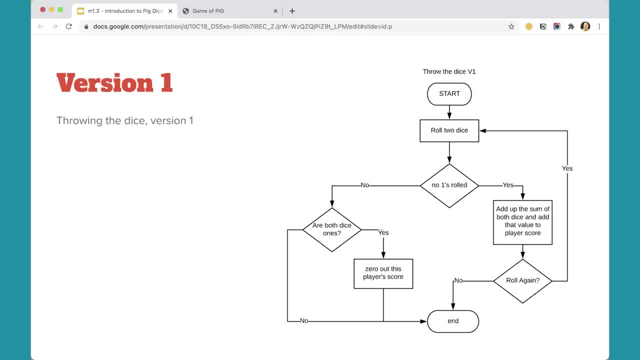 here What happens: Either a one is rolled, either two ones are rolled, or no one, or no ones are rolled. So if no ones are rolled, if that's true, I can take the sum of those dice of those two, die of those two. 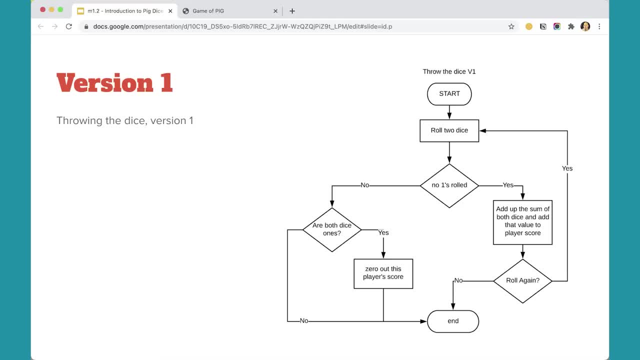 Dice and add that value to my score And then I can decide: do I roll again? If I decide to roll again, I can roll the dice again and I can go through that process again and eventually win the game and end. Otherwise, if I roll the dice and one one is rolled, I can check and see. I can see. 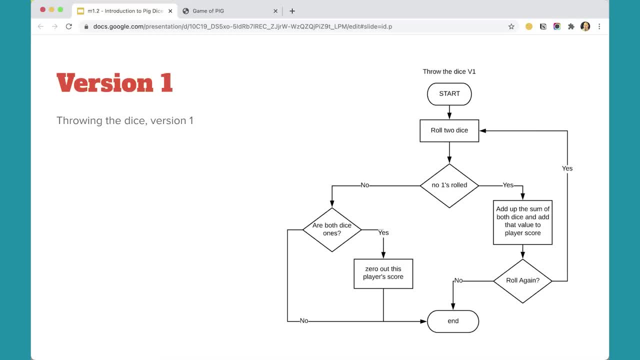 no or or if or if any ones come up, I can see it say: OK, I'm going to follow the no tree there, And then I can check to see are both the dice ones or is just one die, a one while the other one? 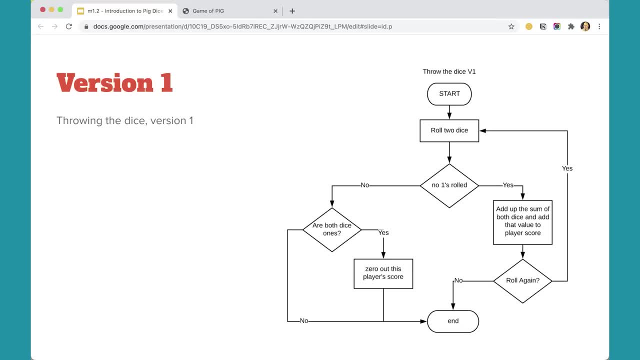 isn't. If both the dice are ones, then I zero out my players score and my turn is over. If neither of the dice are ones that I don't zero out the score, I just end my turn. And that describes the process of a single throw, which, to me, is the cornerstone of this game. 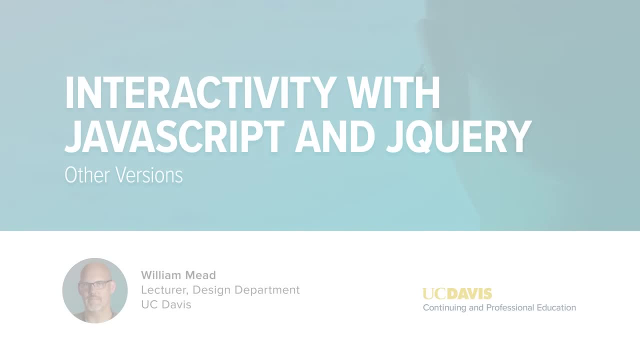 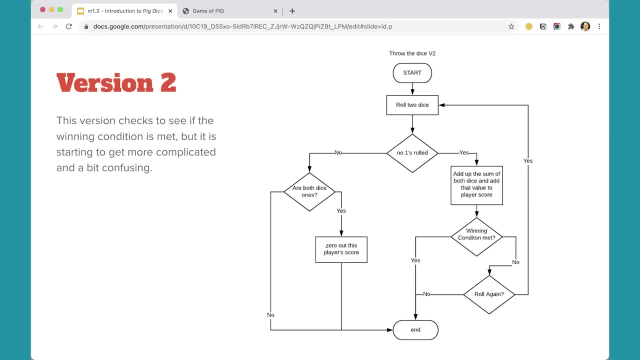 Having done the first version of my diagram, I start to think: well, wait a minute. here I need to keep track of the score and somebody has won, because the game is going to end. It's not just about the throws. At a certain point you're going to stop throwing dice or switching. 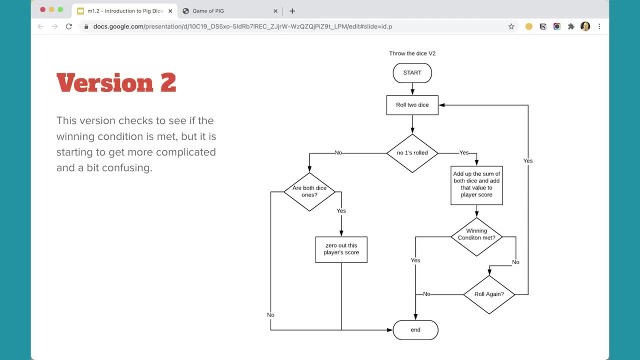 turns And when that happens you're going to check to see if some sort of winning condition has met has been met. So here you can see in the This diagram of updated a little bit to check on that winning condition. I roll the two dice. 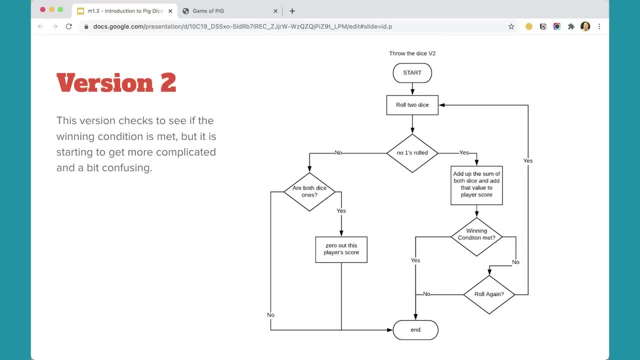 Again check to see if any ones have been rolled, and if none of them have, I can add the score to my sum, the sum to my score, and then I can check to see. OK, what is that total score? and has the 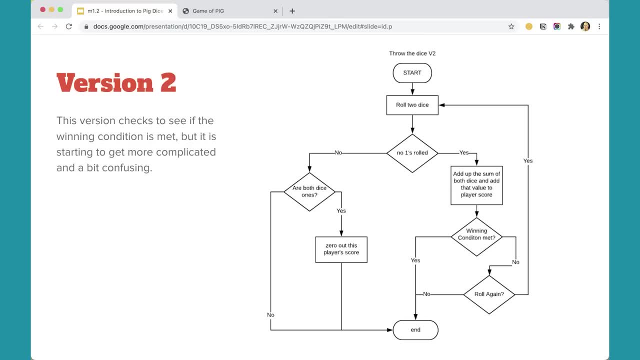 winning condition met in this case, with our rules, the way they're set. Do I have a score that's greater than 30?? And if yes, Then end the game is over. The game is going to totally be over. If no, I can decide whether or not. 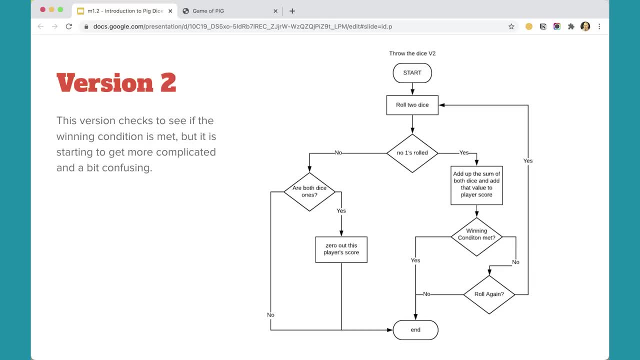 I'm going to roll again, And if, yes, I can roll again, and no, then my turn is over. But the game is not over. So this is starting to get a little bit more complicated and I want to sort of clean up my thinking just a little bit. 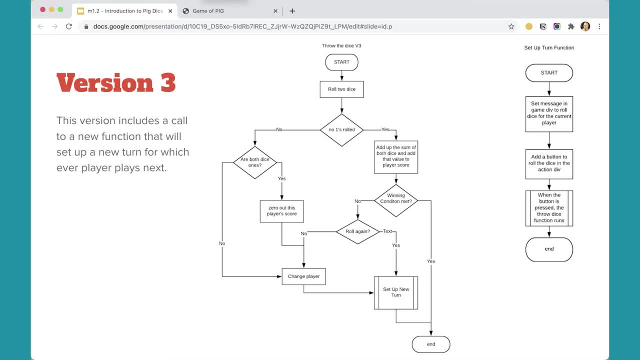 That brings me to version Three of my diagram. here and here in version three you can see that I I start by throwing my dice and I roll the two dice if no ones are rolled, and then I add that sum and I check the winning condition and if the winning condition is not met, I now have a new function called set up turn if 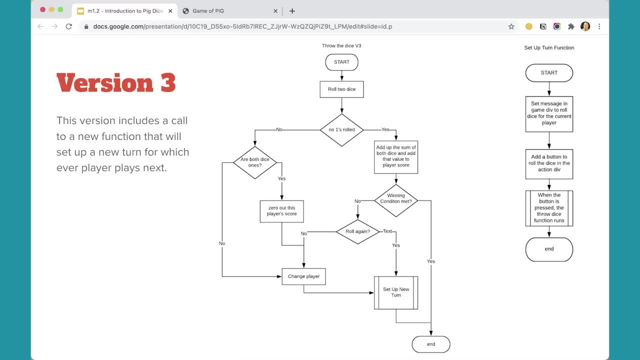 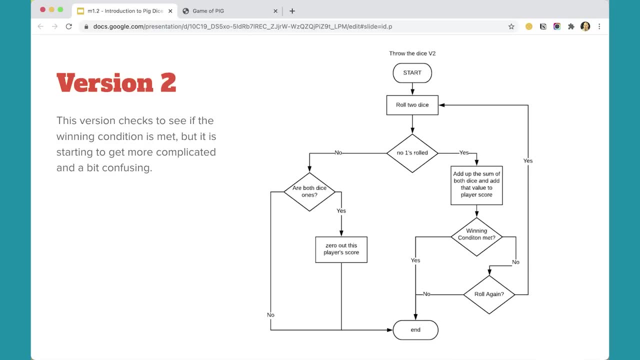 I choose to roll again, So now I have an. I'm introducing a new function in here, because before, in version Two, there was a problem in that, when I end here, if the winning condition is met, this end is representing both the the winning condition having been met and setting up a new turn for the other player. 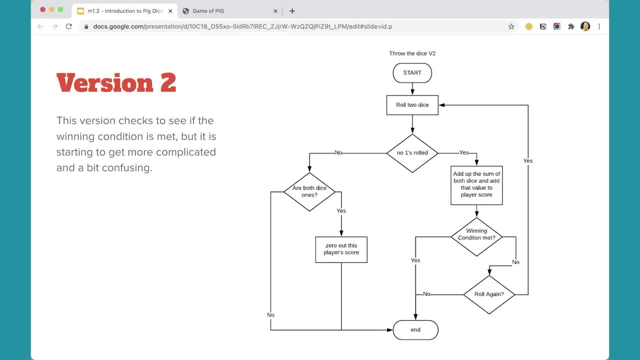 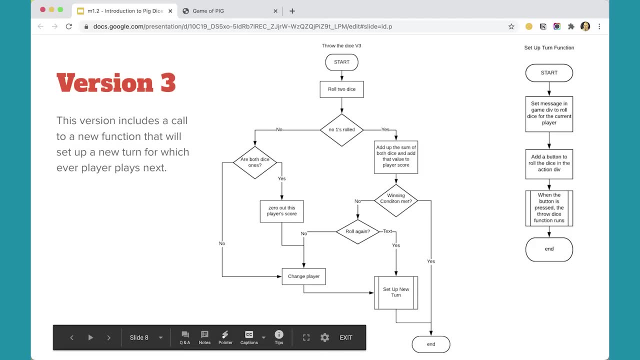 If in fact it's, it's their turn to roll, or I pass, or something like that. So both situations are handled here and I really need to separate those out. So here I've got a new function called set up new turn. So if the winning condition is not met and I choose to roll again, I'm going to set up a new turn. 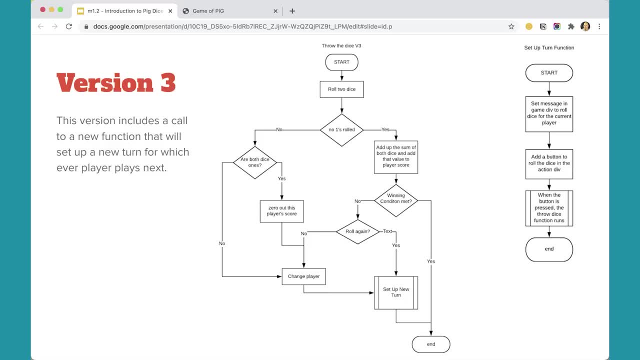 Conversely, if I roll a one and my turn is over, I'm going to change a player and then set up a new turn for that player. So that's looking a little bit cleaner. And now I have a second function here called set up turn function. 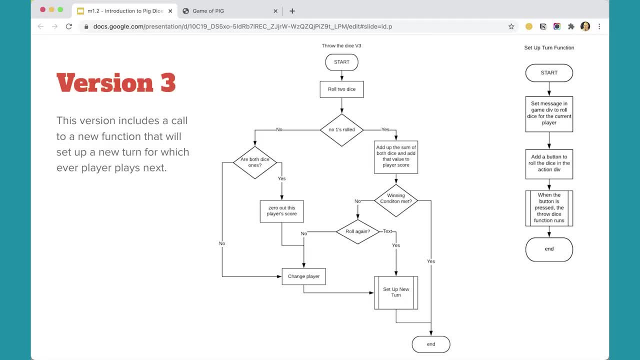 And in this function I'm going to set a message in the game div to roll the dice for the current player. I'm going to add a button to roll the dice for the action div And then, when that button is is clicked, that's when I run this throw dice function that I have on the left. 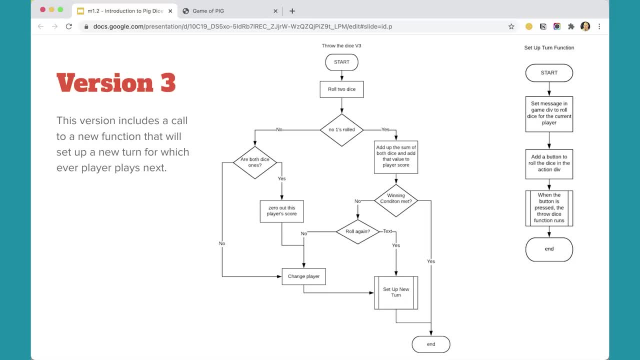 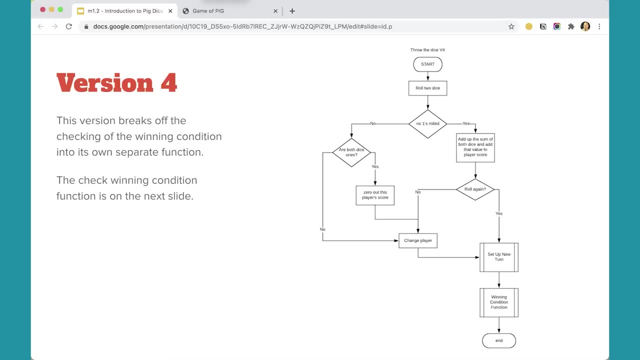 So now I've got a little helper function there that's going to set up a turn, and I've started splitting this out into some different version, into some different pieces here. Version three is still feeling a little bit complex to me, So I decided I wanted to modularize it a little bit more so that now I have a function that's much cleaner. 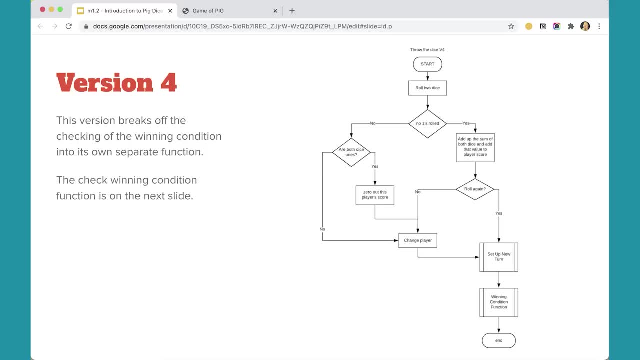 And you can see just by the diagram how much simpler and more clean that it is. And basically what I've done here is I've separated out the winning condition function into its own separately, And then I've added a little bit function that will check to see if I have achieved a winning condition. 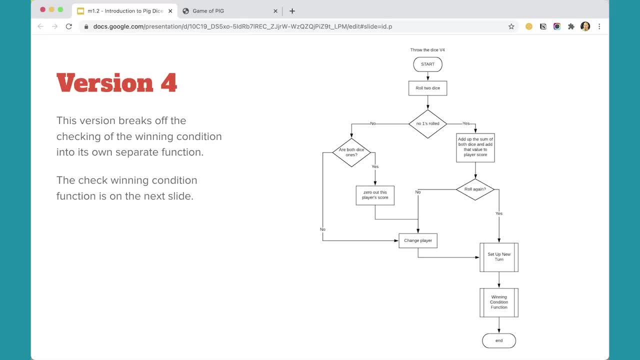 So now this truly represents a throw within the game. You throw the dice, you check to see if a one is rolled. If not, you can add to the score and decide whether or not to roll again. If you decide to roll again, you can set up a new turn and then check to see if you've hit the winning condition or not. 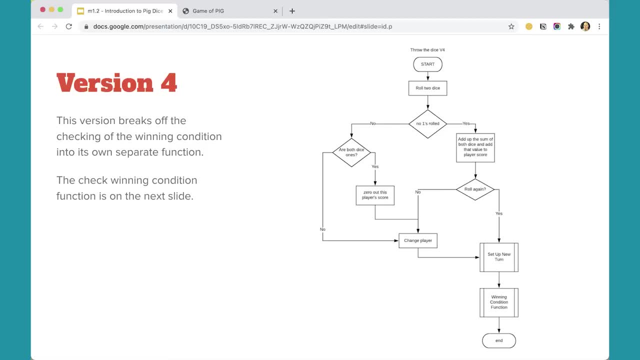 If not, you can change the player and then set up a new turn And then also check to see if it's rolled If the winning condition or not. So this is a much cleaner, much more easier to follow diagram that gives you a sense of what that function looks like. 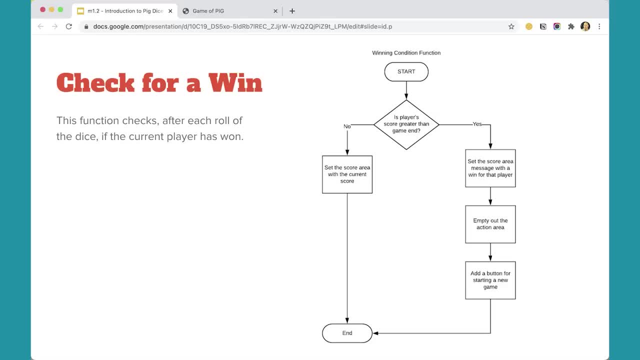 And then we can go on and see what the check for the win condition is. So I start. and is the current player's score greater than the game end? If yes, you set the score area with the message for that win for that player. 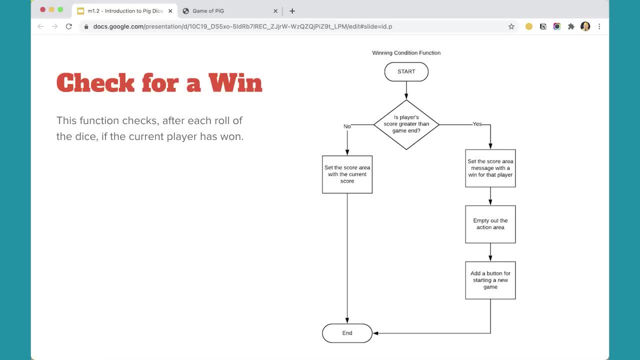 You can empty out the action area and add a button for starting a new game. If no, you can set the score area with the current score, and then you're all set for the next turn. So that's what the winning condition would look like. 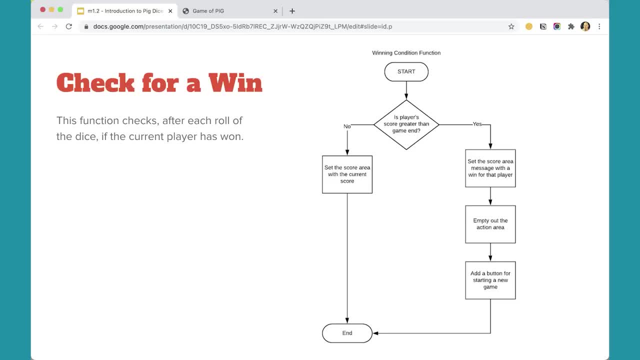 So now we've got three functions that are working together: One that represents kind of the guts of the game, the throw of the dice. One that is about setting up the turn for the next player or for the same player Setting up that next turn. 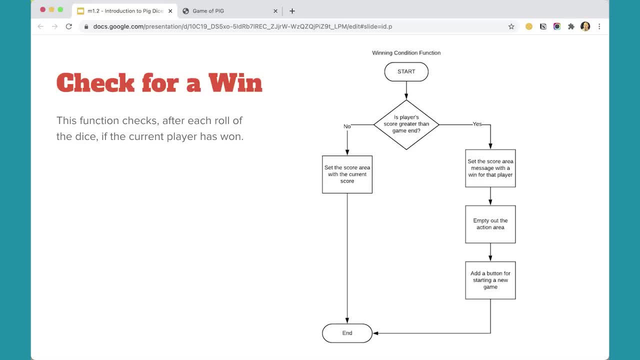 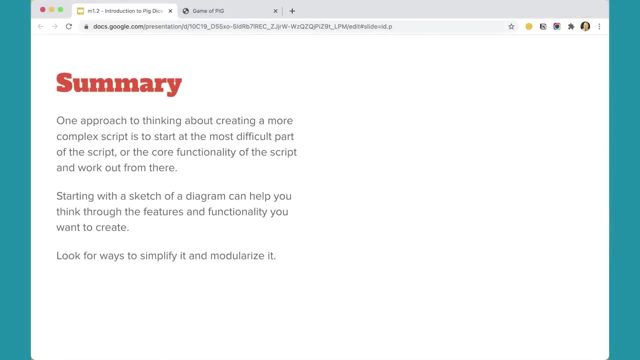 Getting that next turn ready, Getting our board ready, And one for checking the winning condition, And these three functions are going to work together to create this game. So, in summary, one approach to thinking about a game or about creating a more complex script. 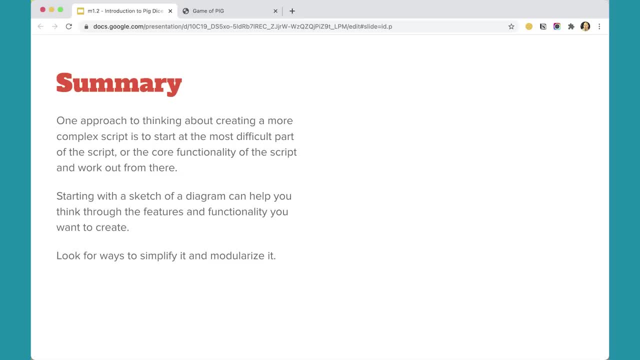 is to start at the most difficult part of the script, or the core functionality of the script, and work from the inside out, And that's what I've done here. I started with the core functionality of What is the core functionality? It's throwing the dice. 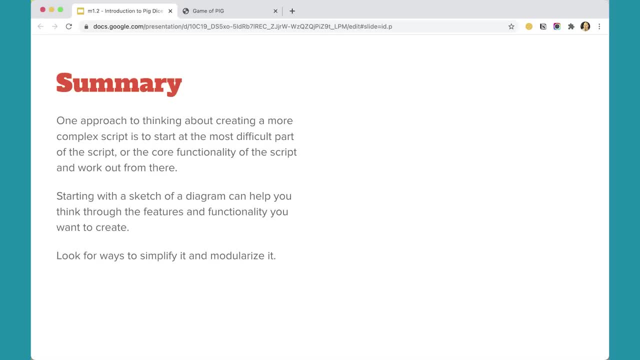 And I worked out from there to think about the score and to think about changing players and to think about other aspects perhaps of the game, And I think doing this will really help you And get better at solving programming problems and taking larger programming problems and breaking them down into smaller pieces. 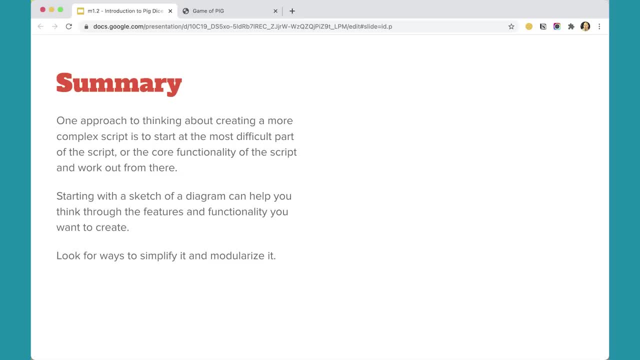 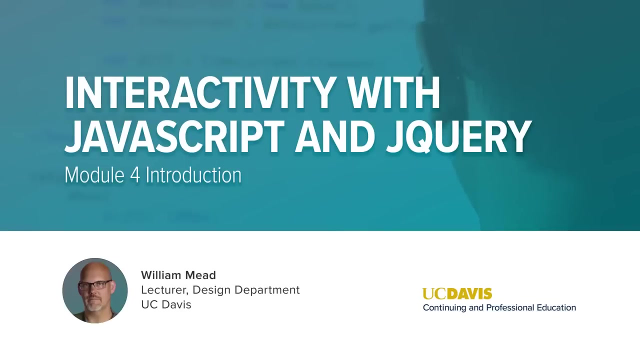 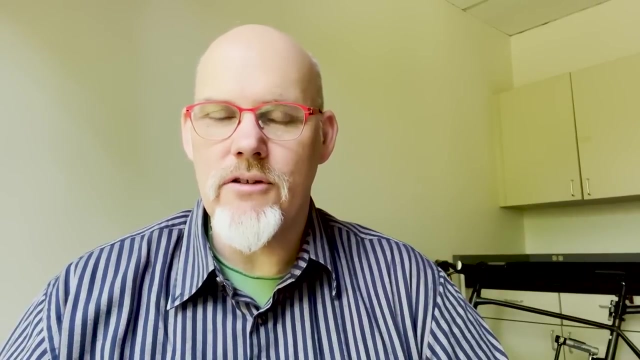 Look for ways to simplify the bigger problems and break them out into modular pieces as much as you can, And to really think about which functionality you need for each piece. Hello and congratulations to making it to the fourth module in our third course on JavaScript. 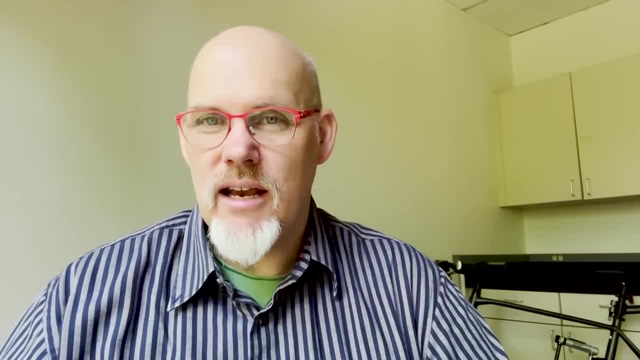 In this module we're going to build the game that we started designing and planning in the third module. I think you'll get a lot out of doing that. It's a fun game And at the end there are lots of ways you can take this game and expand on it. 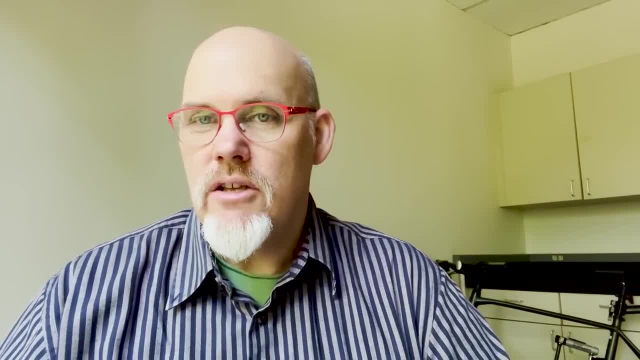 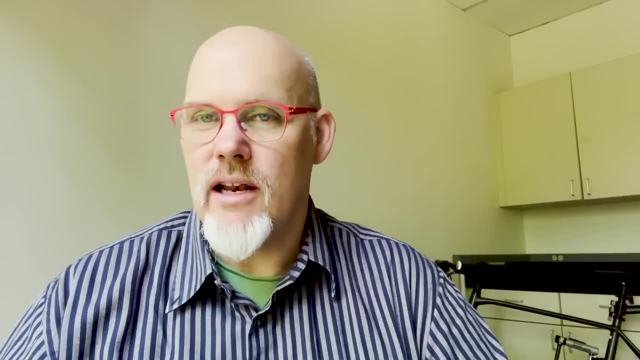 or change the rules or do something different with it. So let's dive in, break out our code editors and our web browsers and have a lot of fun with this project. I've had a lot of fun creating the material for you And I think you'll get a lot out of it. 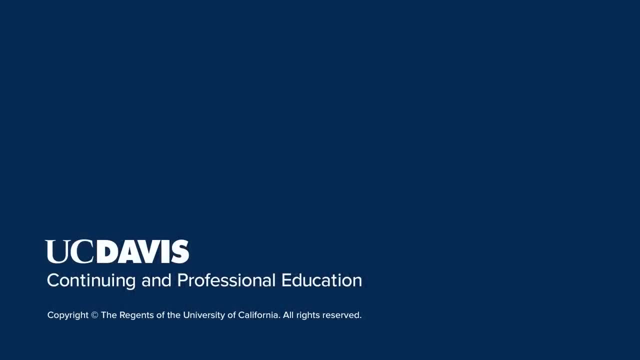 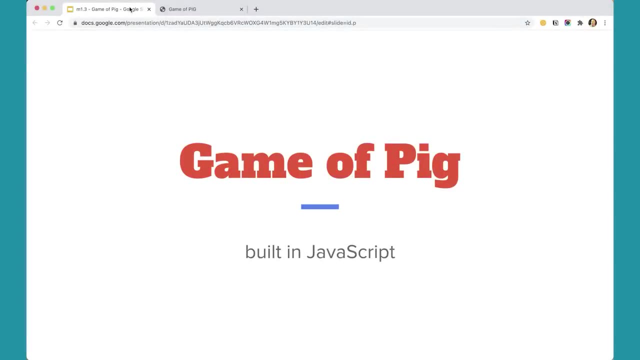 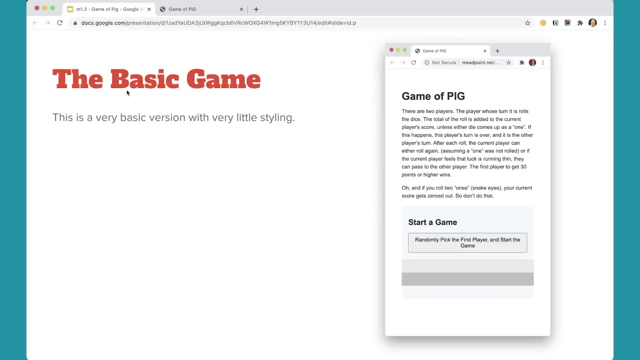 So let's get to it. Game of Pig Built in JavaScript. This is just a very basic version of the game with very little styling, so we can really kind of just make it work. We can go back later and add some better graphics and better styling on your own, if you want to. 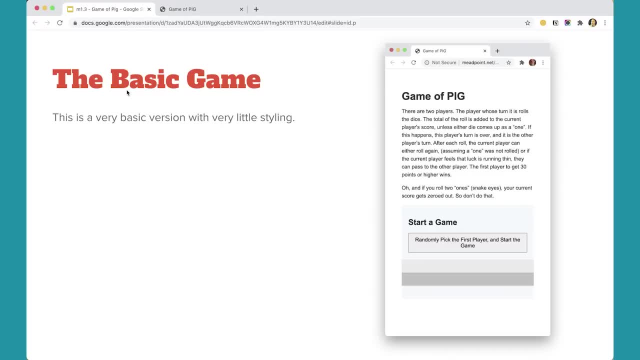 In fact, I hope you actually expand on this game quite a bit and make it your own, And there are lots of ways to do that that we'll talk about later. The other thing that's important to mention here is that the game as we're building it is. 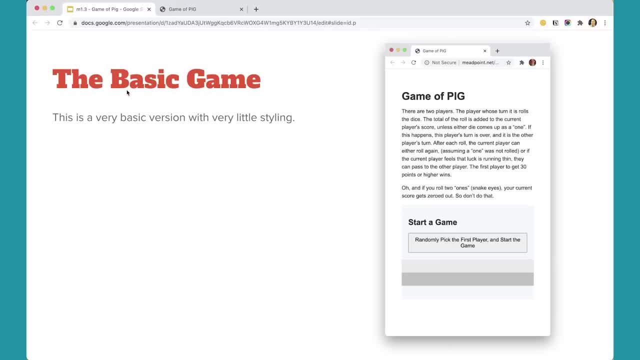 the way I'm going to show you how to build it is in a very linear way, starting from the beginning and going to the end. But from the previous lesson, all you got that. that's not the way I actually develop it or the way many developers work. 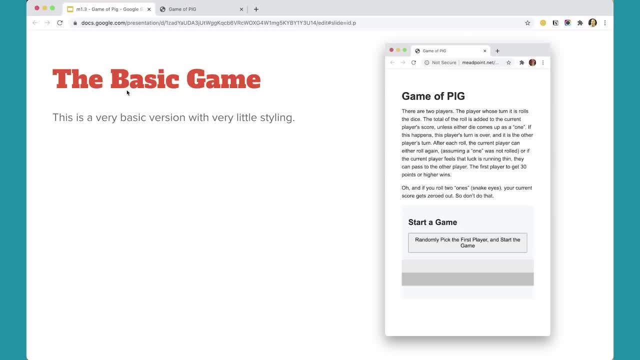 is that they just start at the top and go to the bottom. Usually, you work from the inside out and start with core functionality and work out from there. That's the easiest way to start thinking about. how are you going to solve real problems that are programming problems? 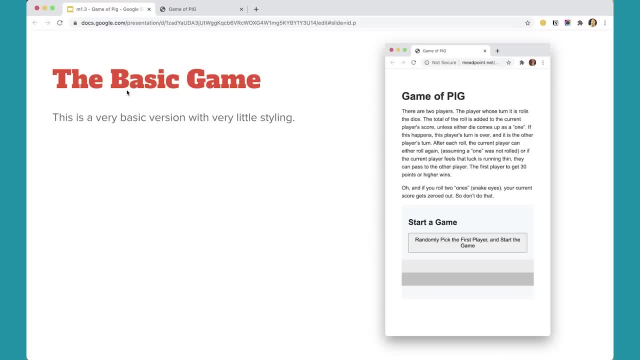 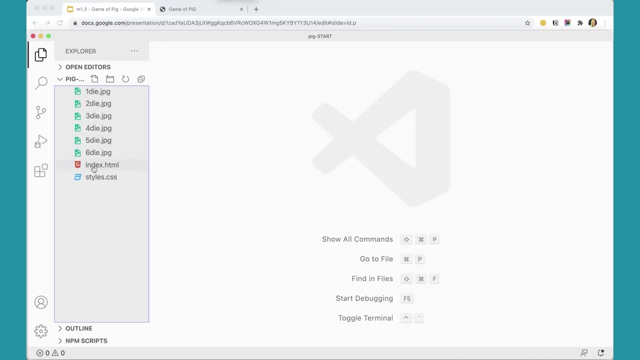 So I'm presenting it in this linear way because otherwise it would be really confusing, But it's important. It's important to realize that it's not developed that way and that people don't necessarily think in this very linear way. I have my file open here in Visual Studio Code. 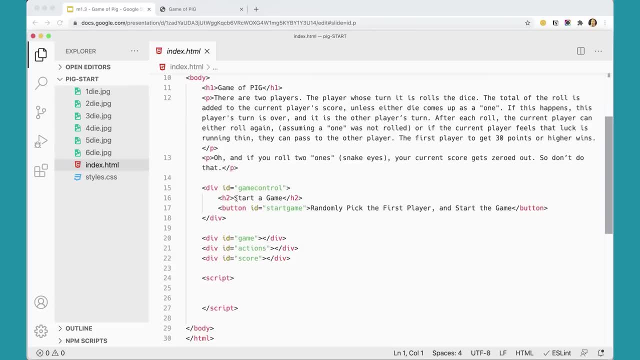 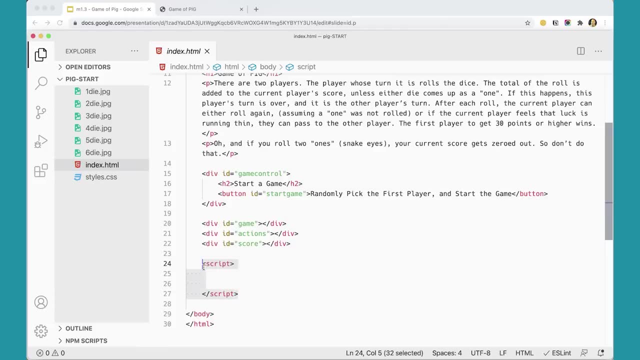 This is the index file here, with all of the basic pieces of the HTML that are needed here to make the game work, And we've got an empty script tag down here, So this is where we're going to be working- is in this part of the page. 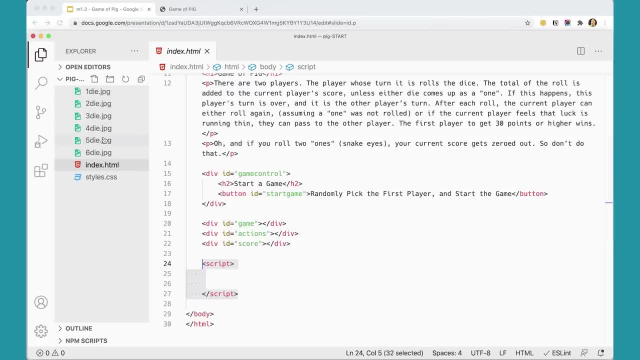 And then also we have the images of the dice that we'll be pulling up. Those could go into a folder, but at this point I just have them in the main folder and that's fine. And then over here I have the page loaded up. 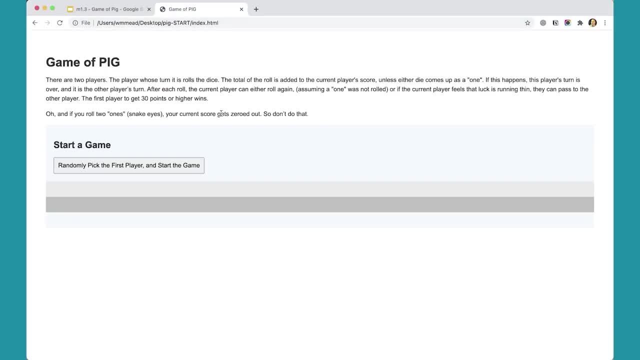 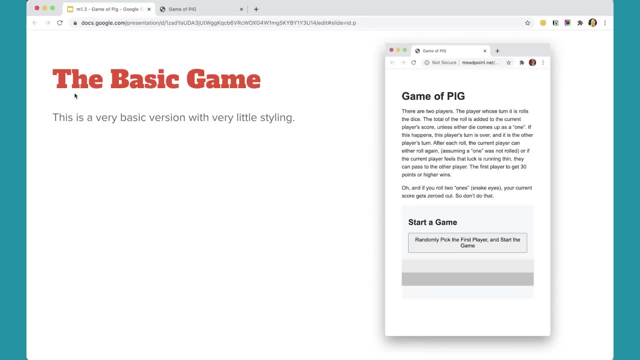 so we can actually test the page here and see how things are working as we go along and work on the page here. Okay, great. So the first thing we need to do in our code editor is create some variables that we're going to use. 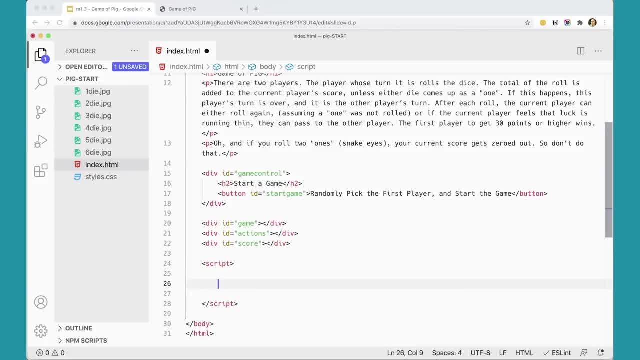 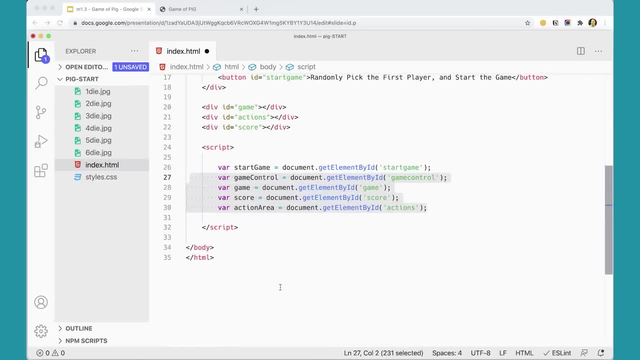 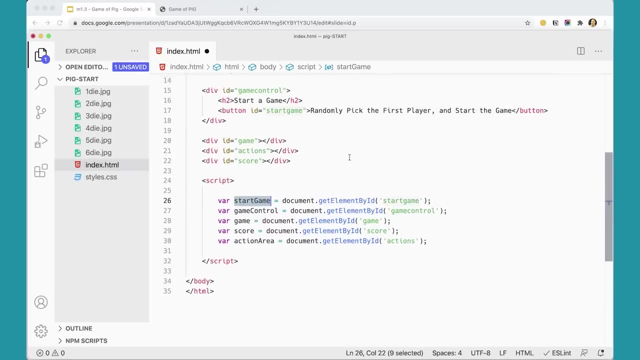 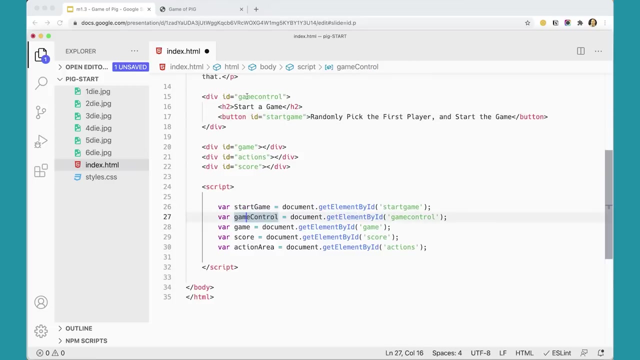 to access different areas of the page. So it's really these variables here. So I'm going to have start game is going to be document getElementById- startGame, So that's this button right here, And then I have game control, which is this whole div. 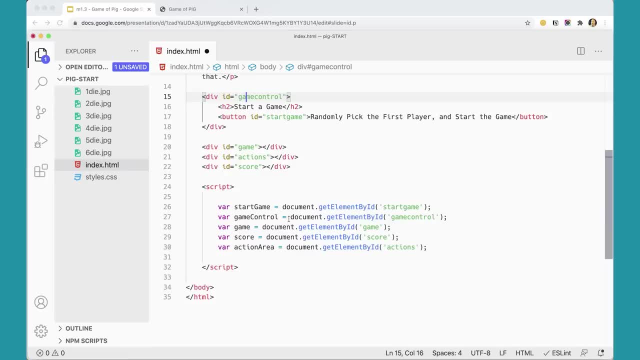 So the game control div. And then I have getElementById. This is where the game is actually going to take place. If you go back to the previous lesson and pull up the game and play it and inspect it, you'll see that that's where the game takes place. 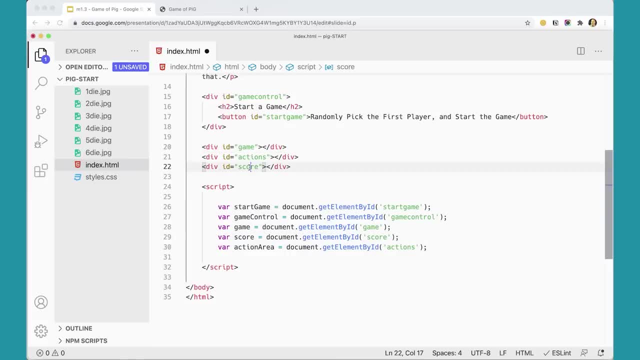 Score is going to be this part down here, And then I have action area, which is this div right here: actions, And it doesn't really matter. These are kind of out of order here, but you could put them in a different order. 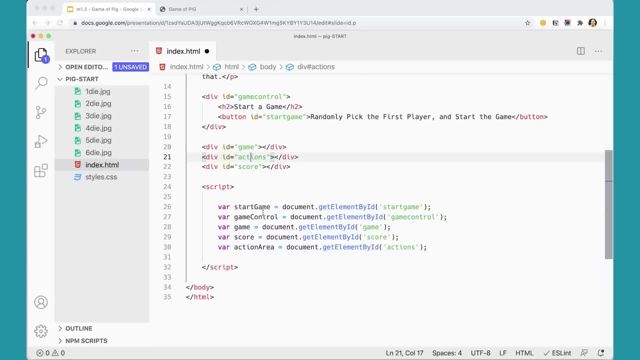 But it's just getElementById. I'm just getting these IDs for each of these elements, So make sure you get this code in here first, because these are the different parts of the board that we're going to need to be able to access within our script. 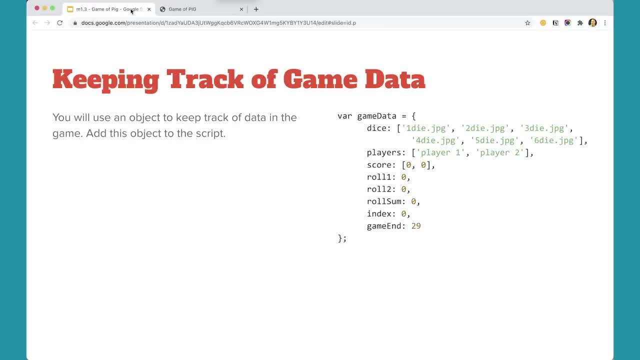 The next thing that you're going to need is an object to keep track of the data in the game. So this is a perfect use for an object. We don't have to use an object. We could use variables for this, But this is a perfect use for an object. 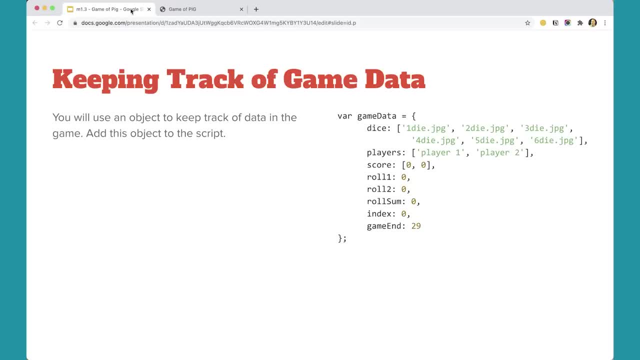 And allows us to practice what we've learned so far with objects and using objects to manage data. And so here I have an object called gameData, And this object has a number of members in it. The first three hold arrays. The first one holds the names of the file names. 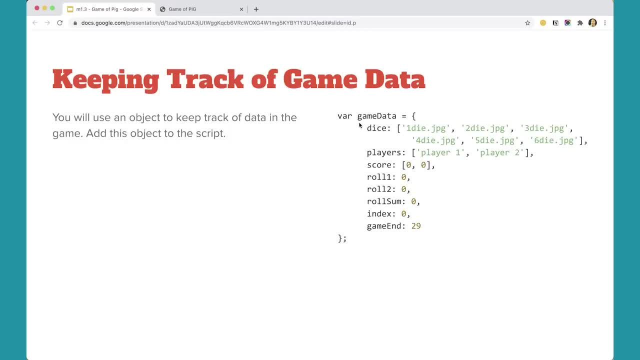 of all the individual pictures of the die. So you know, oneDiejpg is going to have the die with a one dot there. So that's going to be the first one, And the second one is going to have the die with a one dot on it. 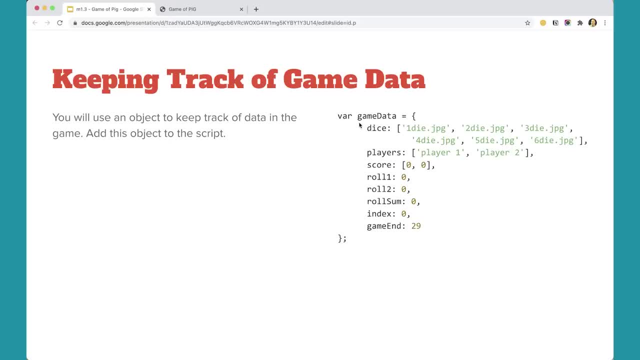 And so on and so forth. The players player one and player two, So those are our two players, So we'll be switching back and forth between those And then we've got a score And that's going to keep track of the score. 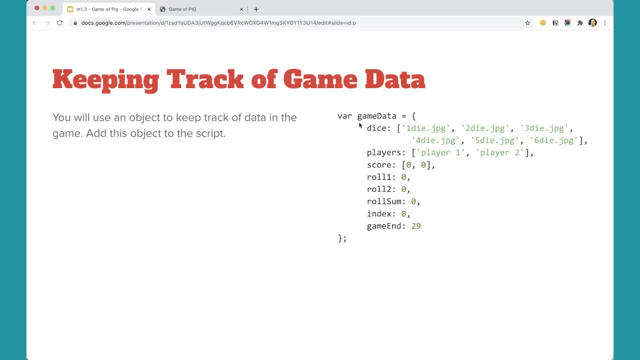 So the first zero is going to be for player one And the second zero is going to be for player two. Roll one is going to hold. each time you roll the dice, you're going to take the number that comes up for that die. 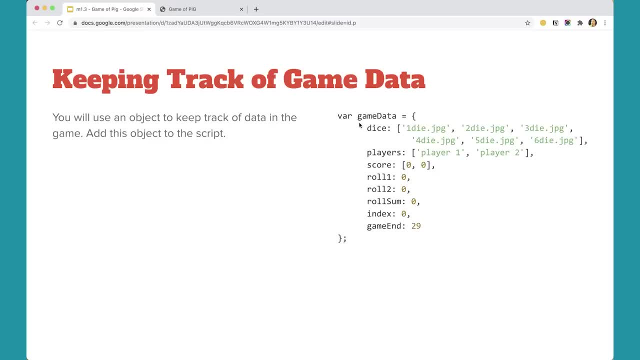 and stick it into roll one. The second die will get roll two And then roll sum will be the combination of both of those together. added together, Index is interesting because we're going to use index. Index is either going to be a zero or it's going to be a one. 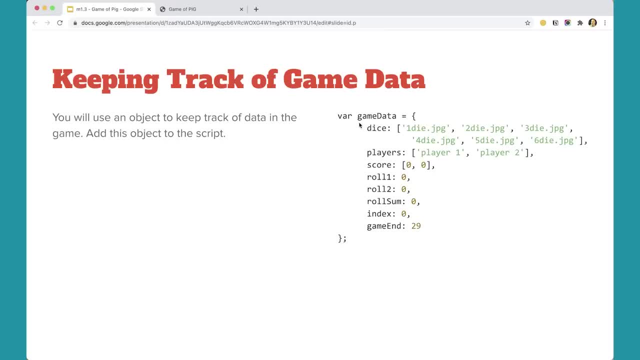 Player one is going to be zero and player two is going to be a one. So when index is one, we're going to use that number one to go into the players array and get player two, We'll be using index one to go into the score. 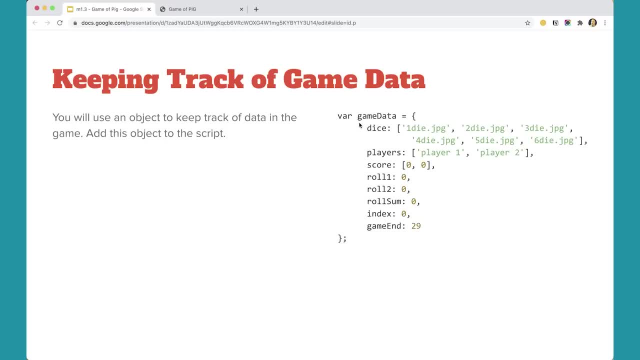 and update the score of that second zero in there And the first zero would be index zero. So that's why we have index here. This is going to change based on which player we're working with as we go through the game And then we've got the game end, which I have currently set to 29,. 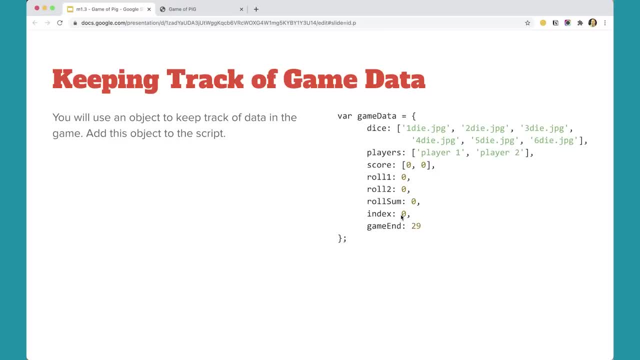 so that you can play the game really fairly quickly and see how it works. Or later you could bump that up to say 100 or something like that, to a score that's maybe a little bit more reasonable for the game. But let's go ahead and get this into our script file. 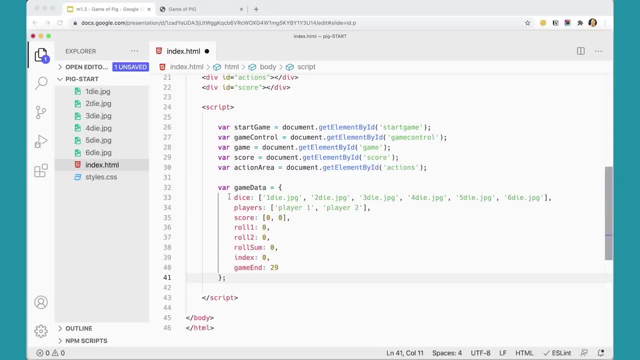 So over here, I'm going to paste it in. You're going to have to type it, but I'm going to paste it in here so that I've got all of these things in here. Make sure you put a comma at the end of each one. 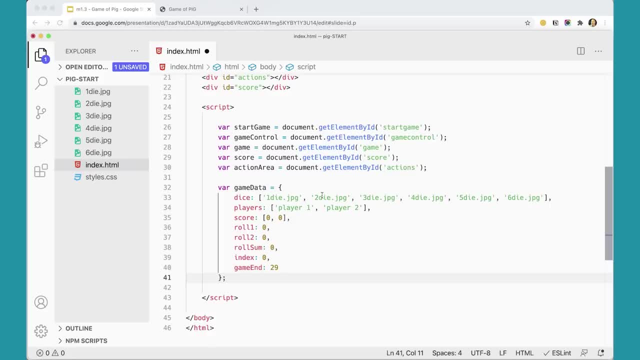 except for the last one. I've got all my dice in here. Notice the comma at the end, But no comma there, Comma at the end here, And make sure everything is right and labeled properly. Okay, great, We're on our way to creating the big game. 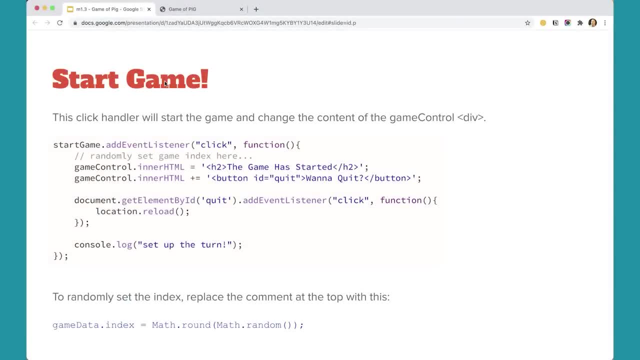 Next we're going to start the game And again, when I was developing this, I started with what happens when somebody throws the dice, But I think for the purposes of building our game from start to finish, it helps to just start at the top. 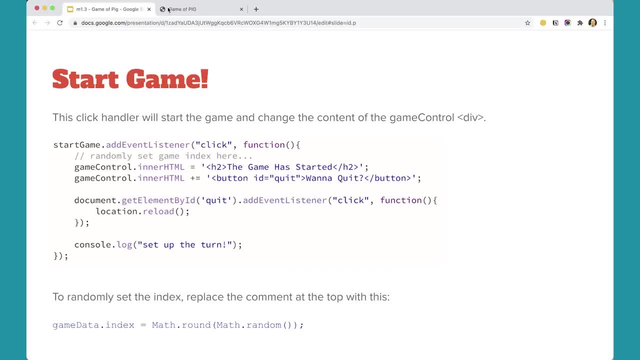 and start at the beginning. So when somebody clicks this button here, we want to start the game, So I need to add a click handler for this button. So that's what I'm going to do here: I'm going to add an event handler for clicking. 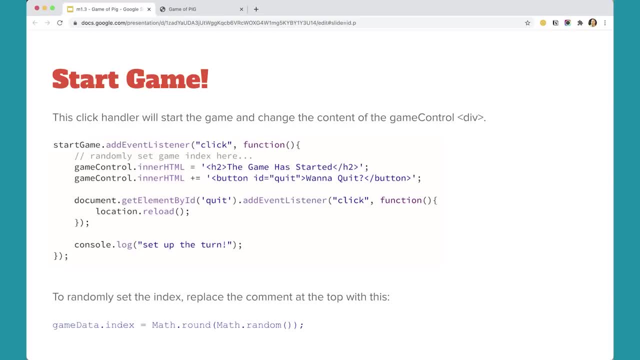 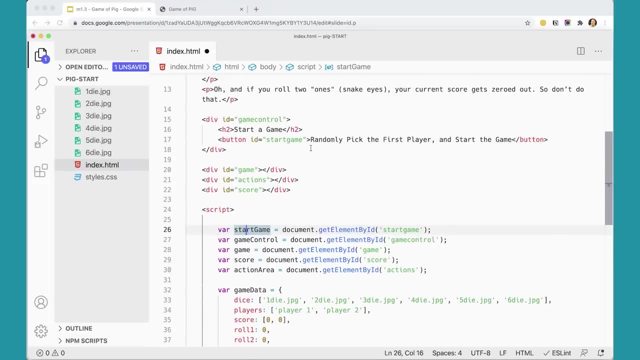 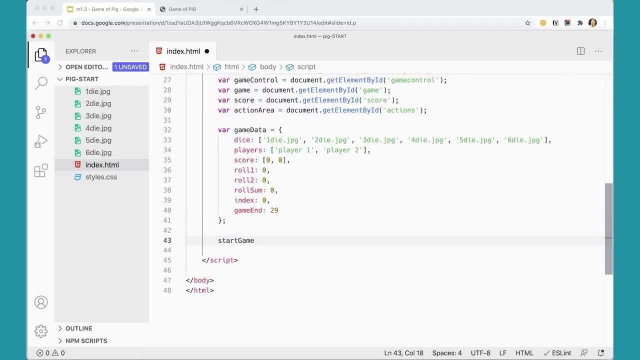 to the Start Game button. So let's do that first. We have our Start Game button defined here, which goes in and gets this button. So we're going to add in our script, we're going to add startGameaddEventListener And we're looking for a click. 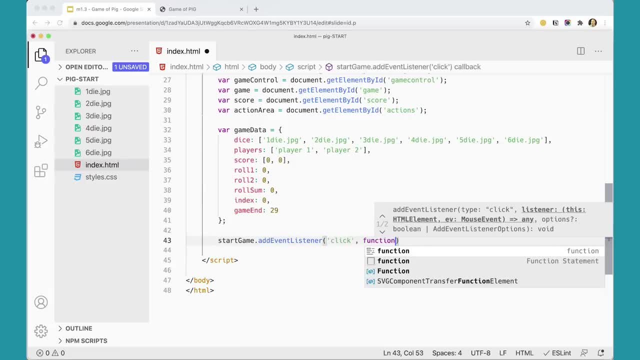 And we're going to run a function Like so And then we're going to put what happens in that function here And we are going to do something with the manager, and I'm going to just put a comment in here now. Change index. 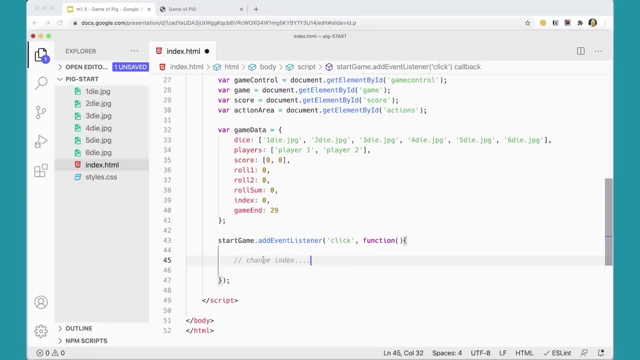 Or randomly select index. Whatever we want to put in there, We're going to have to handle that. But before I do that I want to first just sort of get the correct HTML on the page, So up here at the top of my page. 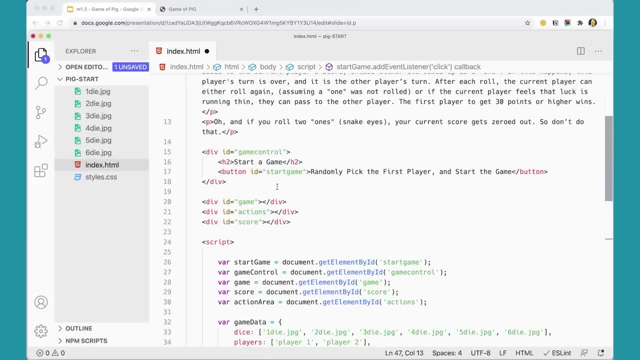 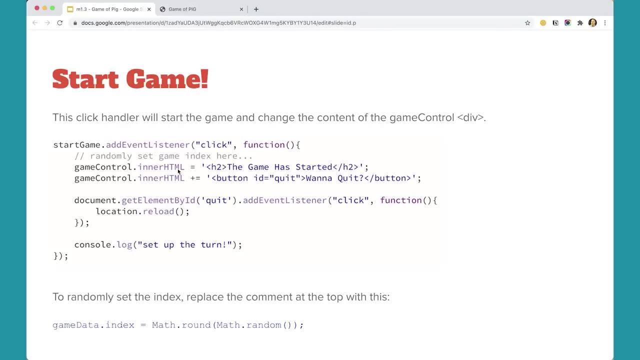 in this section called Game Control here. now that I've clicked the button, I don't really need it anymore And I don't need the Start Game text anymore. So I'm going to use innerHTML to change that Game Control there, So I can set GameControlinnerHTML. 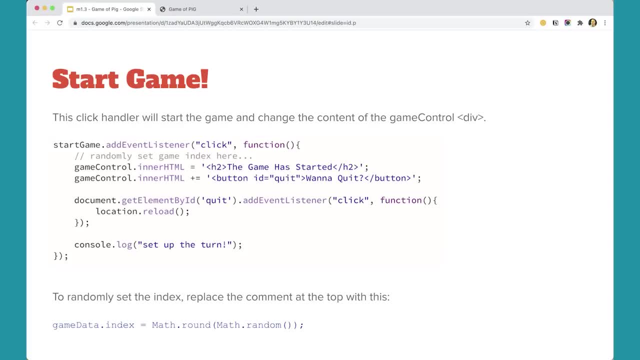 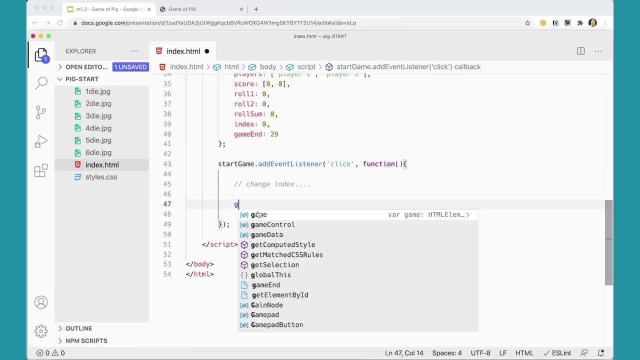 and I'm going to put in just an h2. the game has started, kind of thing, So let's do that. GameControlinnerHTML equals and I'm just going to use single quotes, Single quotes here. h2, whoops, h2.. 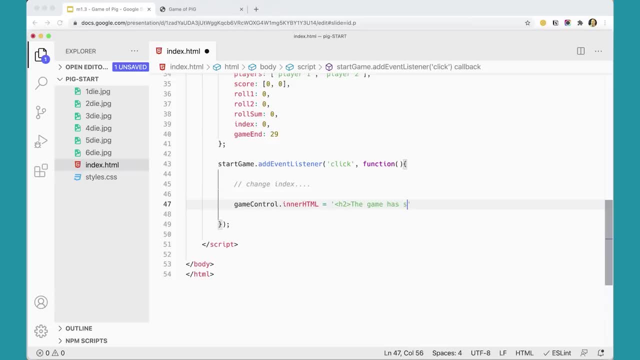 The game has started. You could make those title cases if you wanted to. Might have done that on my picture there, And then I want to also add to that a button, And I could just sort of continue this string here, but I think it's a little bit easier. 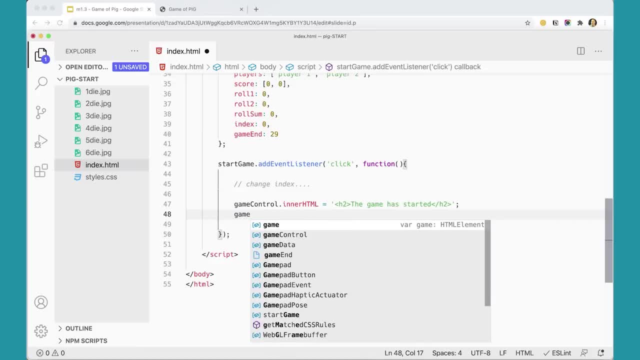 to read. if I just do it like this: GameControlinnerHTML plus equals- Don't forget the plus, Because that's going to add to this string that we already have here And again, I'm just going to put a button And the button's going to say: 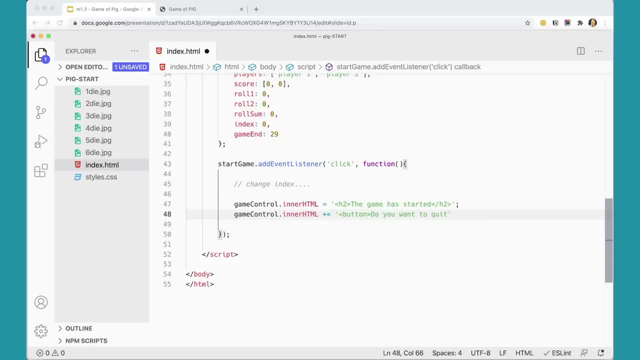 do you want to quit? And I'm going to close the button And I believe I need to give that button an ID. Yeah, we'll just give it an ID. ID equals quote quit. Notice I'm using single quotes here and then double quotes there. 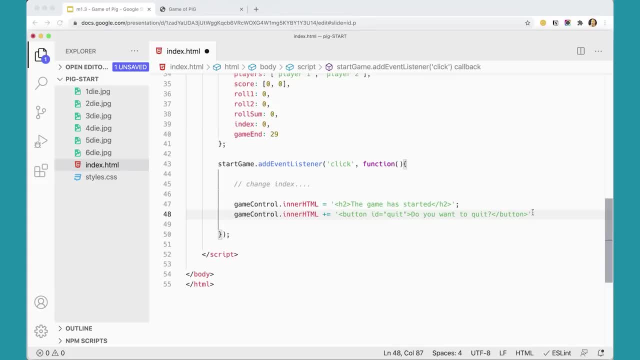 Alternatively, you could use the tick marks on either end as well. Make sure you get your HTML right. OK, So we're going to add that in there. That's great, And now I just need an event listener for when somebody clicks the quit button. 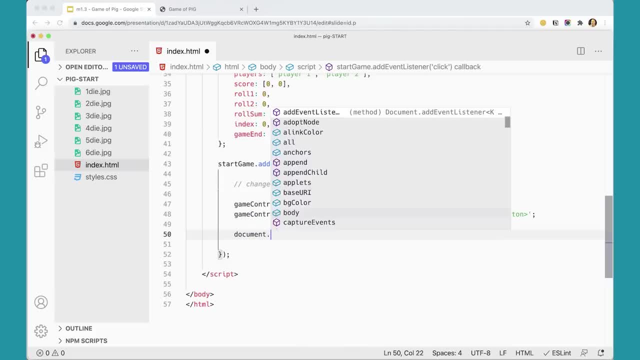 So I'm going to say documentgetElementById- quitaddEventListener. When you click that, we're going to run a function like so. And what's going to happen in that function? We're just going to do windowreload, I believe. I'm sorry. 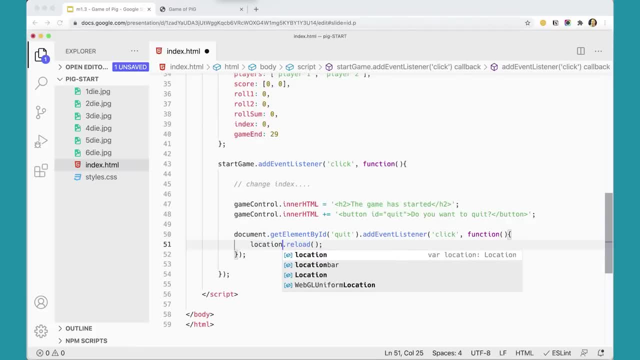 I'm sorry, It's locationreload And so that basically just refreshes the page and then you go back to the way the page was before. OK, great. So when you click the button, these things will happen and we'll get that working. 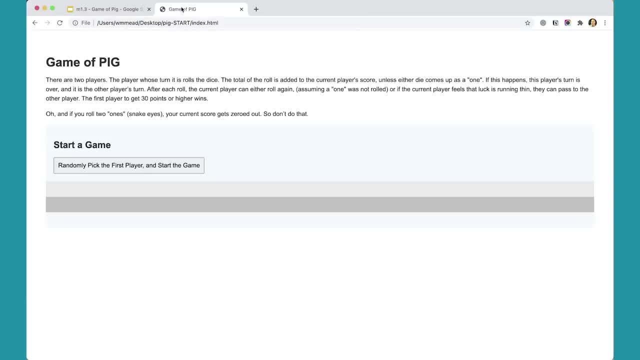 Let's just test this much and see if it works. If I come over here, click refresh, When I click that we get the game has started. When I click do you want to quit? it just refreshes the page and puts it back. 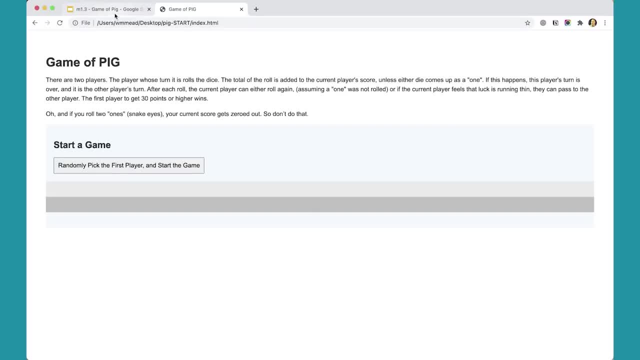 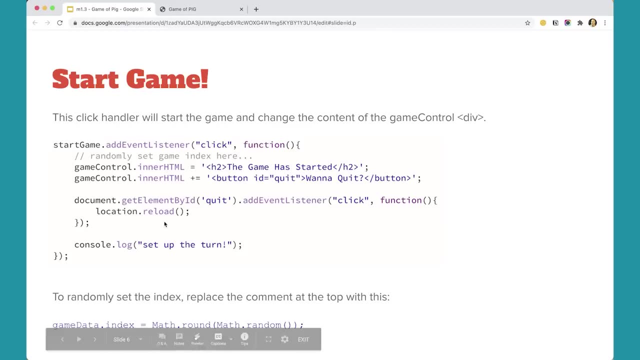 So that's working just fine the way it is. We're going to test as frequently as we can there. Now the last bit is: I also want to set that game index, the gamedataindex. I want to set that so that we can see. 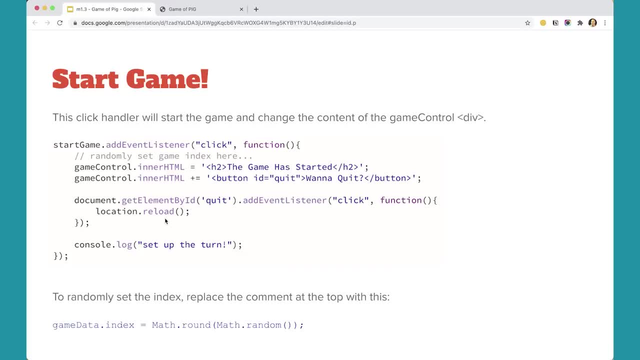 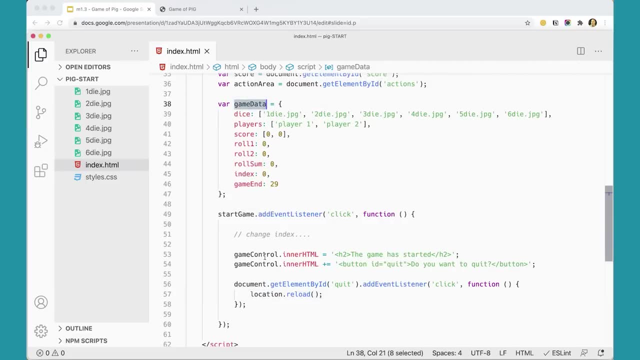 that we're getting a random player. So gamedata is this object here, And so I'm going to actually say gamedata, gamedataindex. This element is going to equal mathrand And that will actually round, I'm sorry, mathrandom. 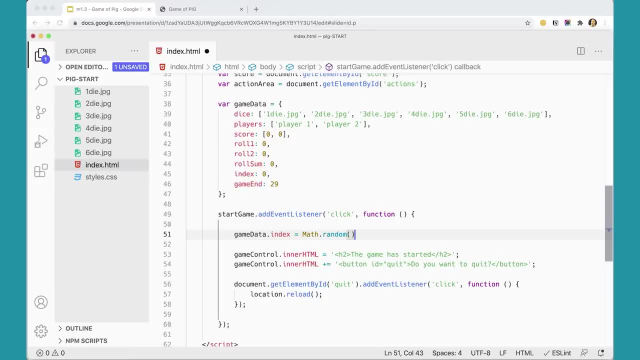 That will actually generate a random number of zero and one, And I want to round it because I want it to round up to either one or down to zero, because I want index to be a zero or a one, So I can do that on the same line here. 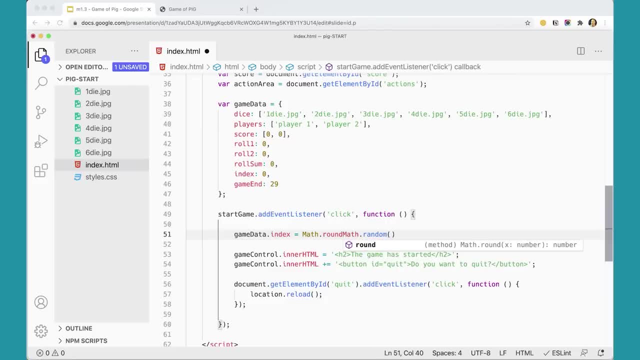 by putting mathround and then surrounding that. So mathrandom will pick a random number from zero to one and mathround will round it up or round it down. Let's add a console log so that we can really see what that's doing. consolelog- gamedataindex. 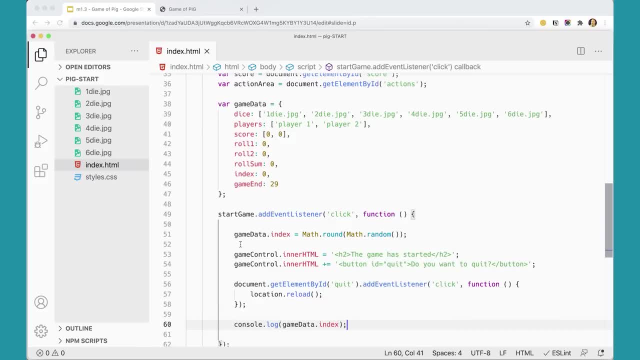 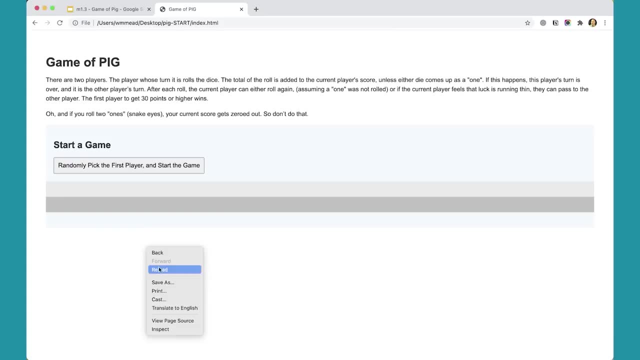 What is the value there? And we'll test that and see. So let's come over here and I'm going to refresh the page. I'm going to turn on my inspector so I can get to the console log consolerandomly and I got a zero. 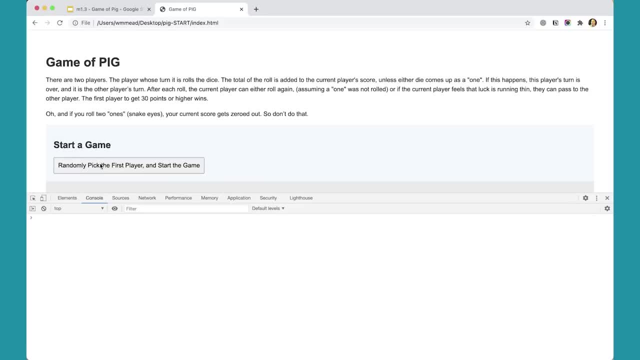 If I click on acquit and pick again, I'm getting zero each time. here, There we go. now I got a one. So it's either a zero or a one that's coming up, And I'm getting one a bunch of times. 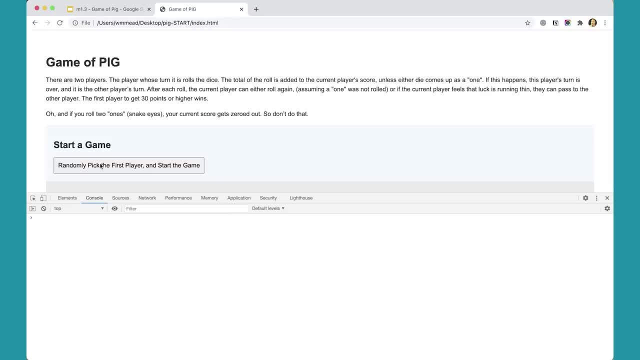 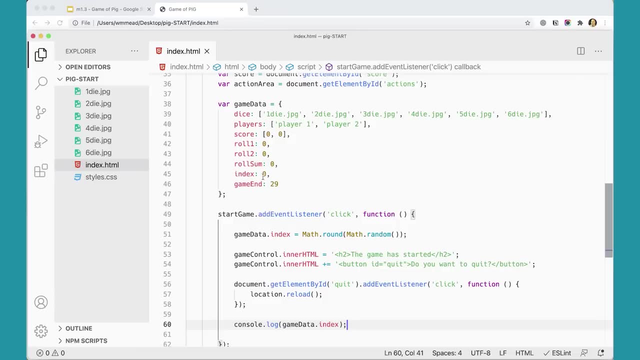 So each time you start the game you're either getting a zero or a one, So that will pick one player or the other. So hopefully you can see here that index being a zero or a one, is going to choose player one or player two. 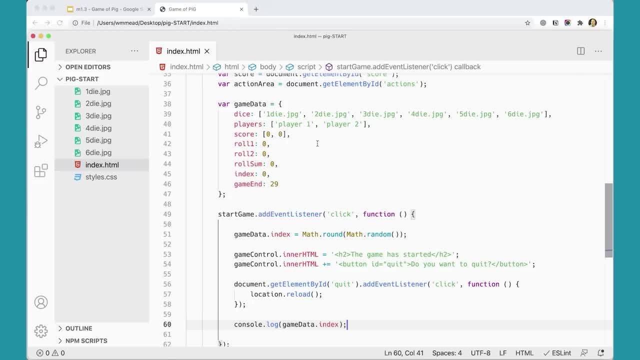 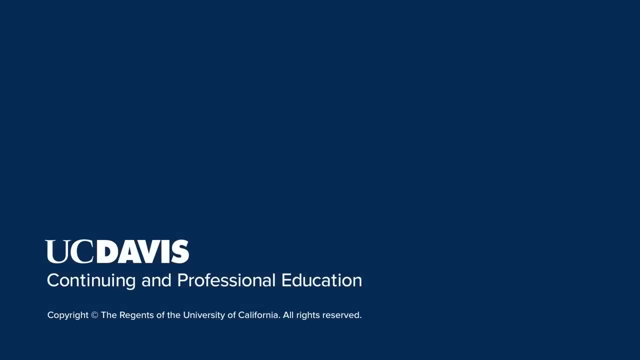 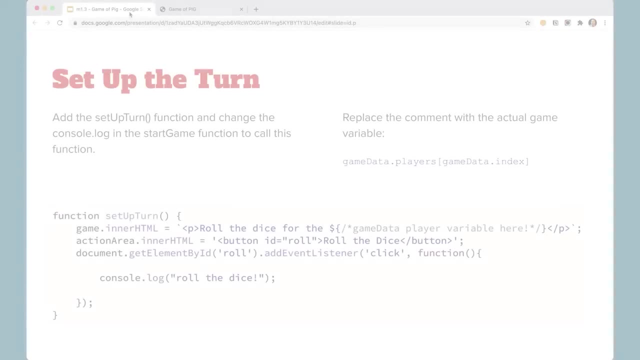 This is zero, this is one. Okay, great, We've got a good start at making our big game. Let's keep going in the next video. The next thing we need to do is set up the turn, So we're going to create a function for that. 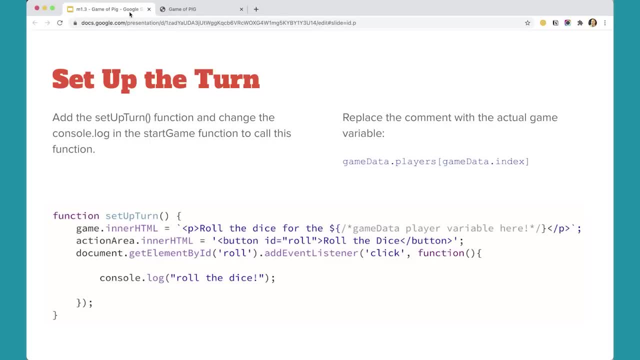 And remember, we're going to have three basic functions in this game. One of them is set up the turn. We're going to have one for rolling the dice And then we'll have one for checking the winning condition, And it's really the way these three functions work together. 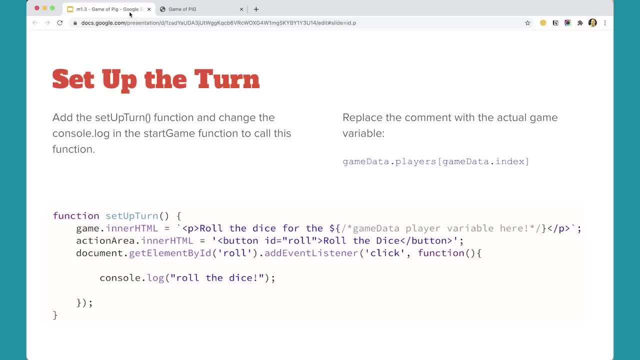 that are going to determine how this game works. So the first thing we're going to do is really is the set up the turn function And in that function we'll take game and we're going to set its inner HTML to roll the dice for the correct player. 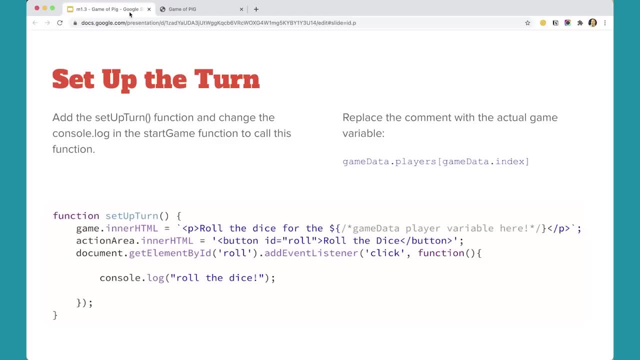 And we'll fill that in as we go here, And then we're going to get that action error. We're going to set its HTML with a button that allows us to roll the dice, And then we'll have an event listener for that button. 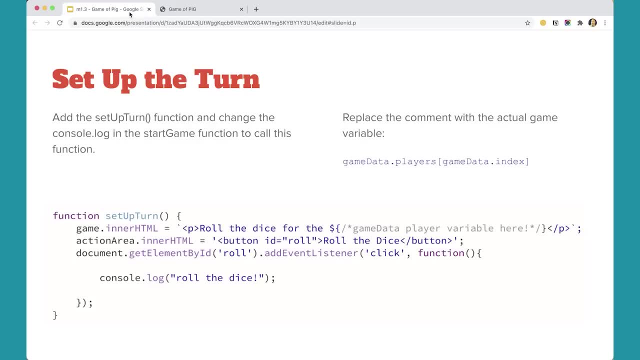 so that when you click it it will actually roll the dice. And at this point we're just putting a console log in there just to make sure that the button's working. So let's go ahead and add this to our code over here. 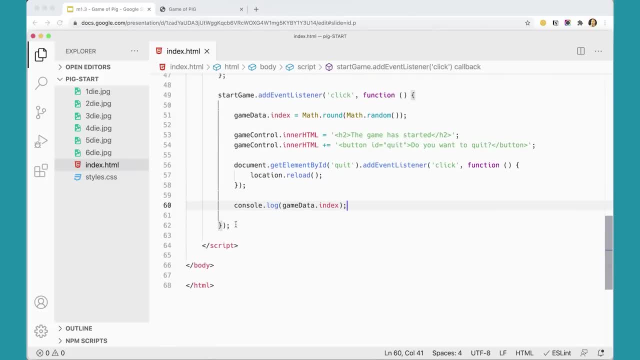 So down here we've got my start game event listener. After the start game event listener, I'm going to add function, set up turn And the first thing I'm going to do here is gameturn. Enter HTML equals and I'm going to use my tick marks here. 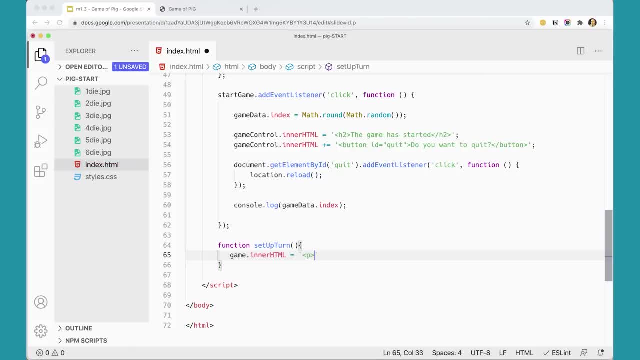 And in there I'm going to put in a paragraph, And you have to use the tick marks because I'm going to include a variable in here in a minute. Roll the dice for player X, Something like that. is what that's going to say. 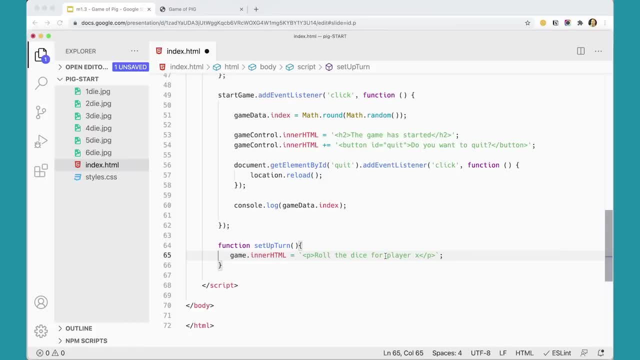 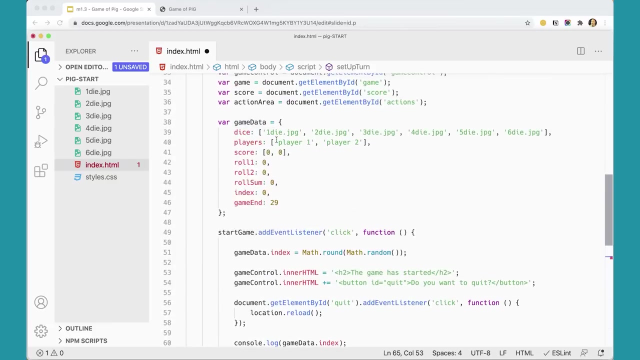 But player X? who is player X? Instead of player X, I'm going to have a dollar sign and curly braces, Oops, curly braces, And in there I'm going to put my game data, game data players and the index. 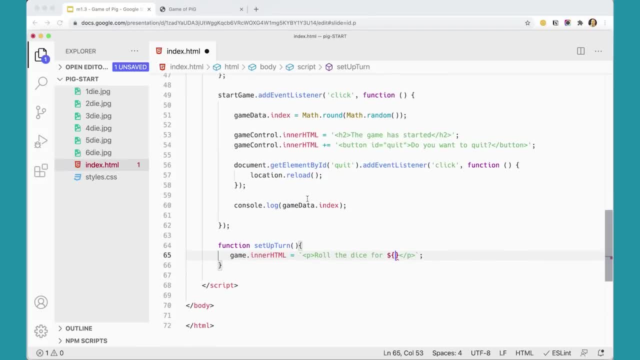 Right, Because that's going to tell me which player I had selected, whatever value got set here for our game data index. So it's going to be game data, game data dot players. And remember players is an array, So that's going to have square brackets. 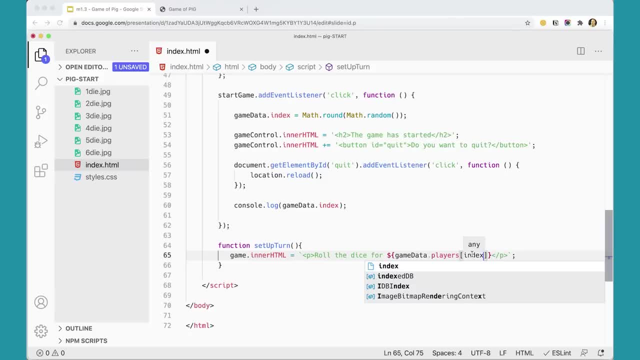 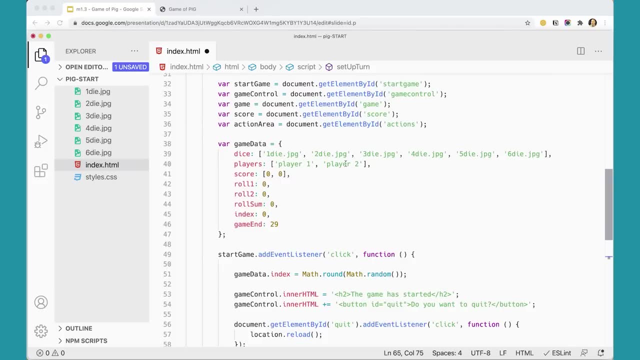 And I'm going to put index in there And that will go in And index is going to be either a zero or a one, So that should go into my game data. find players and get either a zero or one based on which number was rolled here. 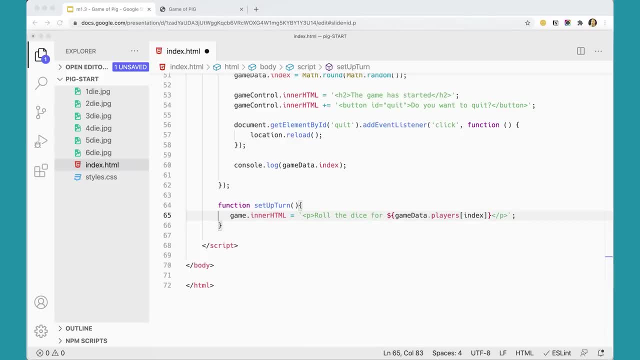 Oops, I'm sorry This needs to be game data dot index. There we go, Because I need to go back into that object: game data dot index. Game data players. game data dot index And that will get that player. 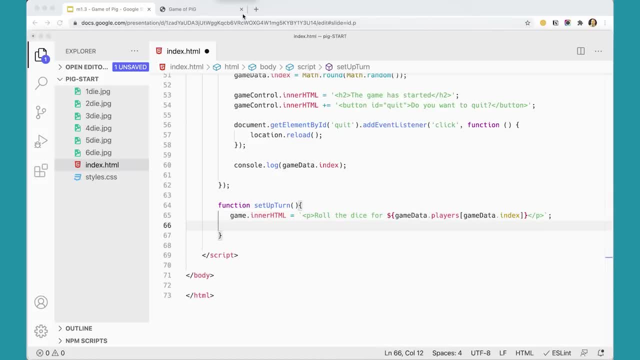 Then we have action area Dot, inner HTML, And this one can just be a straight up string. So I'm just going to use the single quotes here and put in a button with an ID set to roll And I'm going to say: 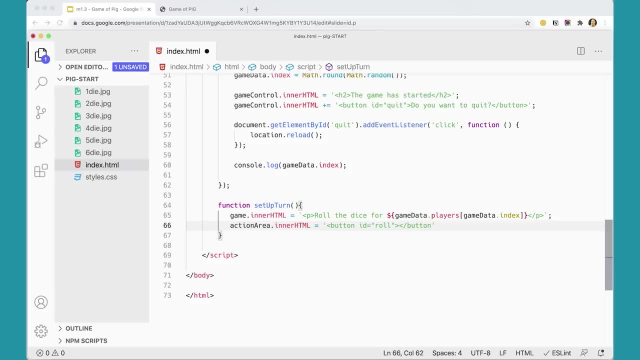 and sometimes it's helpful to close that right away button Like so, And then it's going to say: roll the dice, There we go. So we've got a button that gets added in to our inner HTML for the action area. 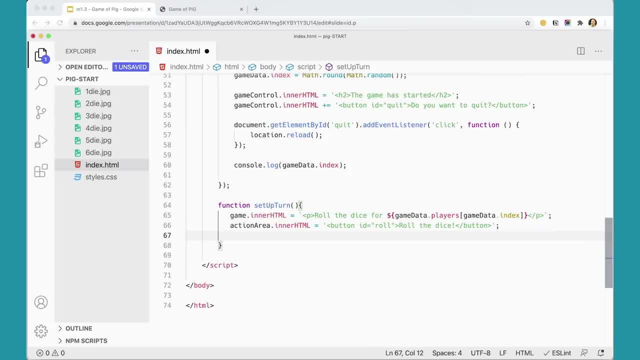 Okay, So we've got a button in the action area. Now we need to have a click handler for that. So I'm going to have document dot. get element by ID roll dot. add event listener Click When we click that. 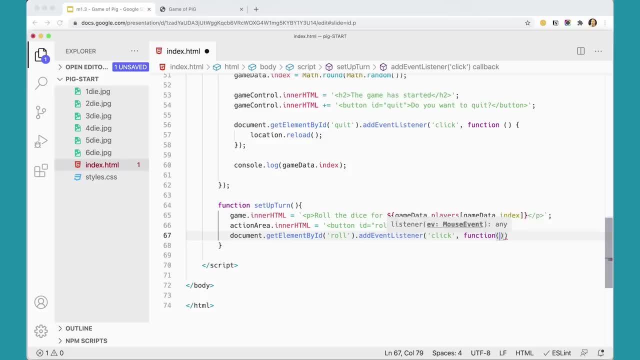 something's going to happen. We're going to run a function Like so, And what are we going to do in here? For right now, all we're going to do in here is console log, console dot log, roll the dice. 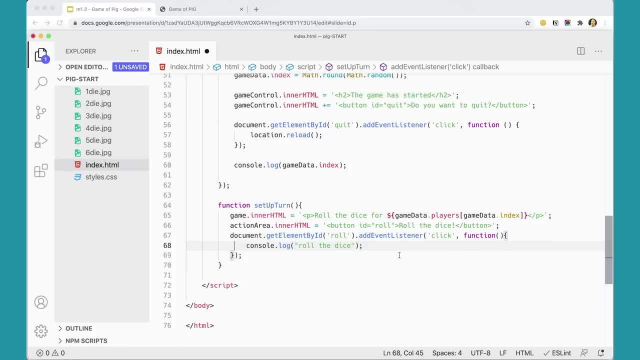 And we'll replace this console log In a few minutes, But that'll give us a sense of whether or not this is actually working. So now, when we've selected the player up here, we now need to set up the turn. So I'm going to run. 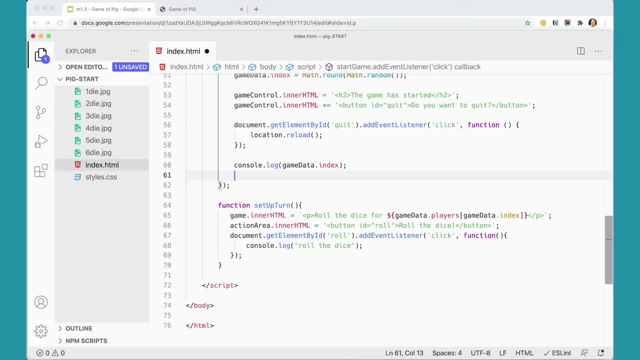 set up the turn here And we can leave this in here for now, for the moment, just for a moment to see if that's going to work. But we're going to run. set up the turn there So that we can get ready to roll the dice. 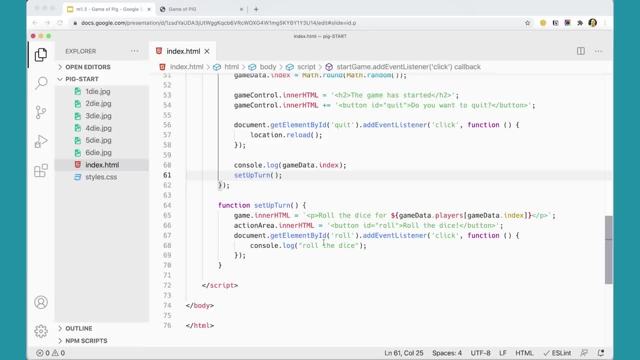 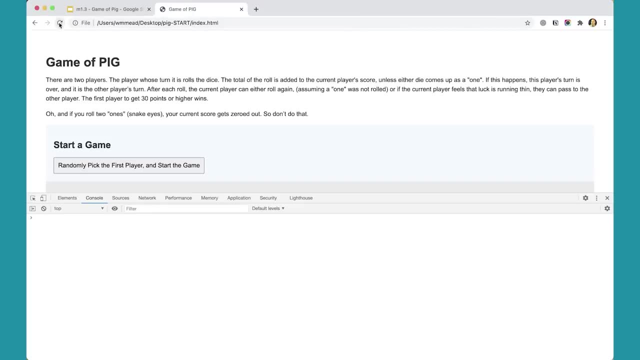 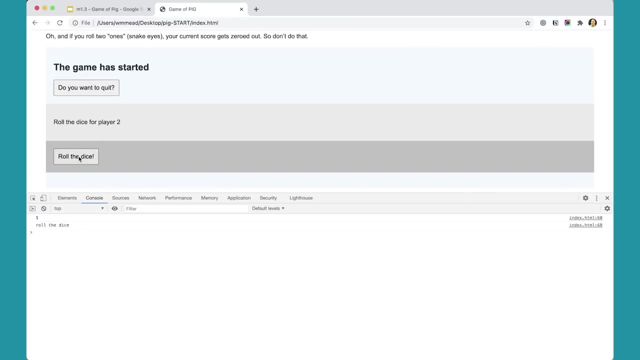 and see how that works. Let's test it. If we come over here and refresh the page randomly, pick the first player, roll the dice for player two. I get a button. when I click it It says roll the dice If I click. 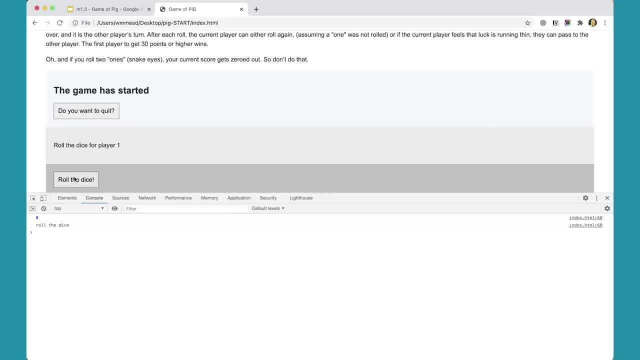 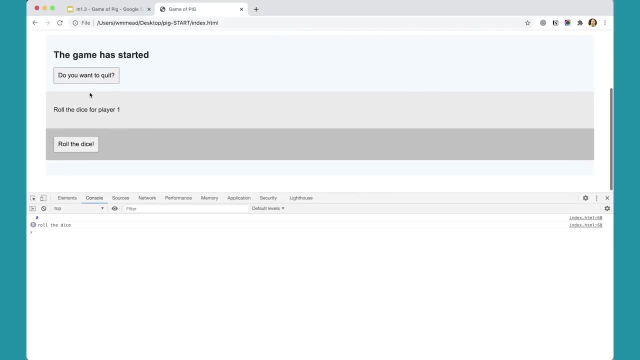 do. I want to quit. It'll go back and I can start again, And at this point, just rolling the dice will just keep giving me more of these. But that's working perfectly. We're rolling the dice, We've set up our turn. 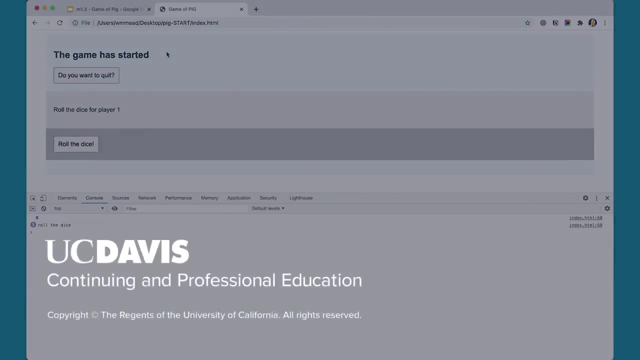 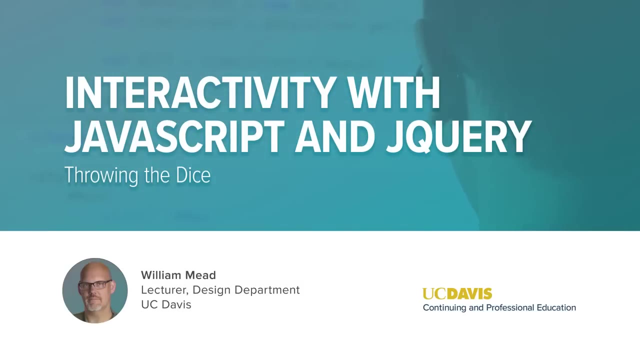 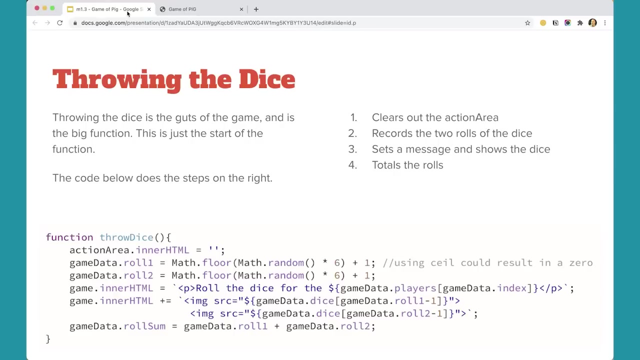 and we're ready to roll the dice, Throwing the dice. So this is the core function in this program And it's kind of the big function. It's going to take us some time to kind of get this function all working, But we're going to get it started here. 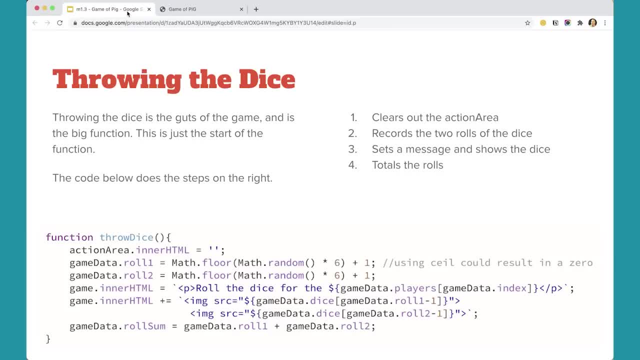 And at this point what we're doing is we're going to clear out that action area, Anything that's in that action area. we're just going to clear it out And then we're going to record the two rolls of each die. 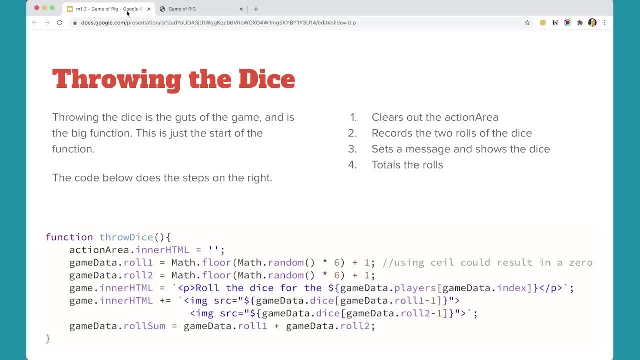 The dice, Record the two dice, Record those rolls into our game data object And then set the inner HTML for the message that's going to go to the player about what was rolled, And then and also show those two dice, And then we'll also sum up the total of those two dice. 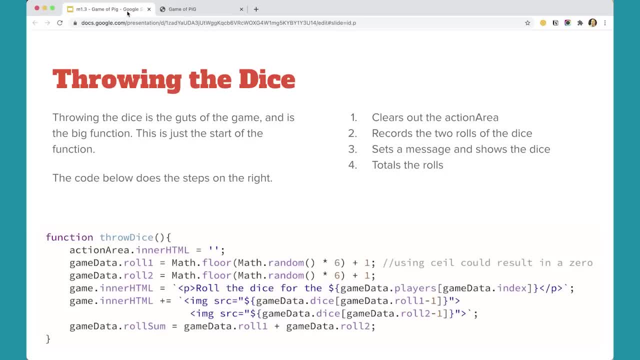 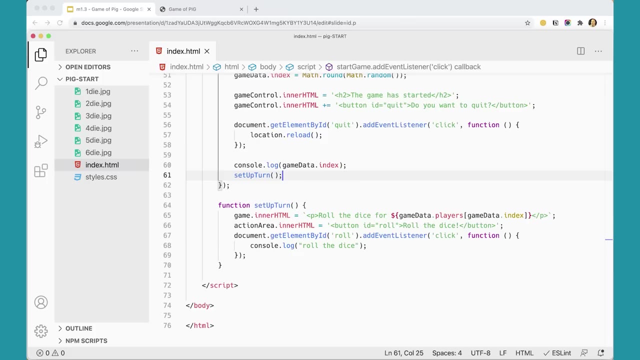 and put that into the roll sum, into the roll sum property in the game data object. So let's go ahead and get this started, because this is an important one to do. So I'm going to add a function Function: throw dice, parentheses, curly braces. 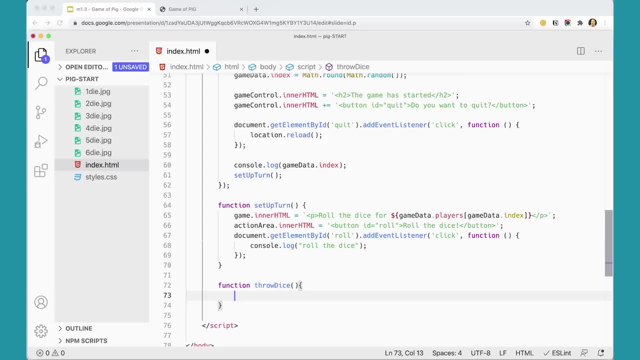 And then in here, first thing I'm going to do is set the action area equal to quote, quote: just empty. I want to clear it out: That's action area dot inner HTML. I forgot that. Inner HTML Action area. inner HTML equals. 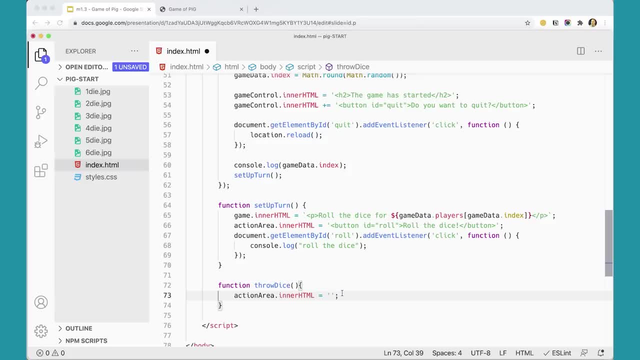 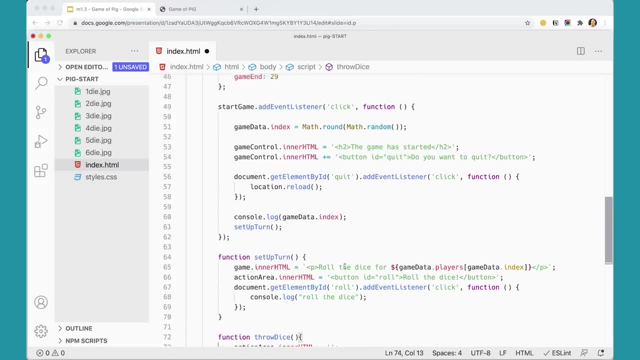 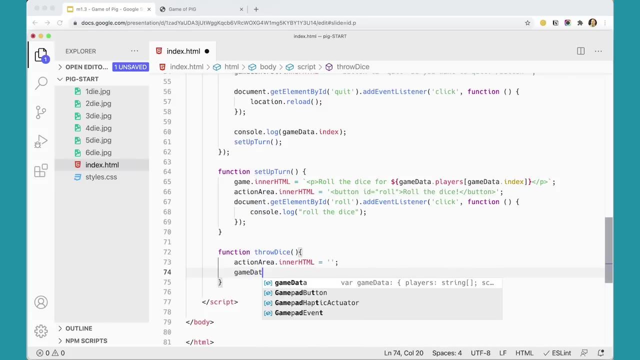 quote, quote. Empty it out. Clear that out. Okay, Clear out that action area. Then I need to create, then I need to set my, my values for my dice up here. Roll one and roll two. So game data dot, roll one. 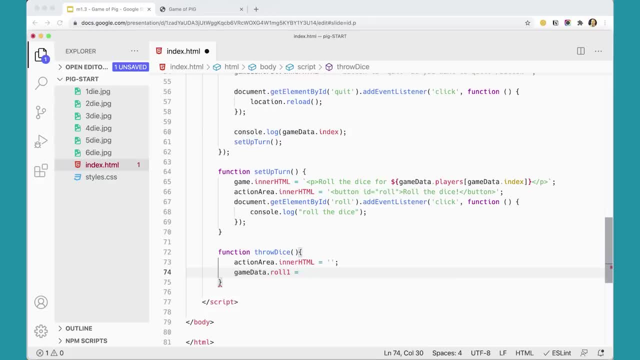 is going to be equal to: and again, I'm going to do a random math dot. random. That will generate a random number between zero and one. But if I multiply it by six and then, and then I need to round it down. 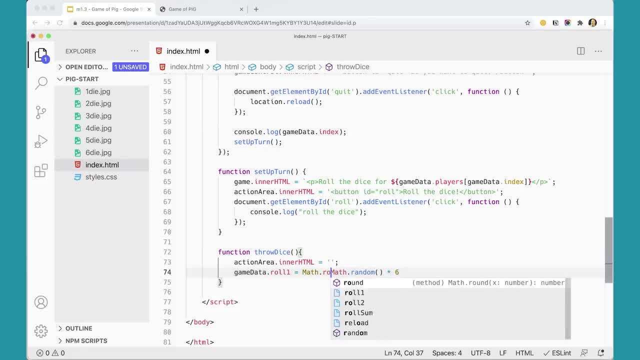 Math dot, math dot round. Actually, I want to do without floor And then I want to add one to it, Because what this will generate is a random number That's basically between zero and five. So I want a random number because my dice are one. 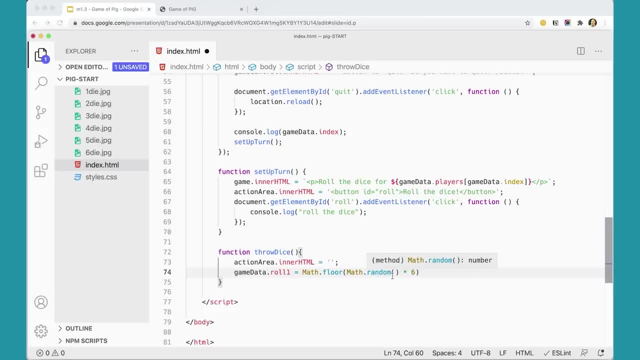 two, three, four, five and six. I want a random number, That's a one, two, three, four, five or six. I'm going to add a one to that, Plus one. Now, you might wonder here: 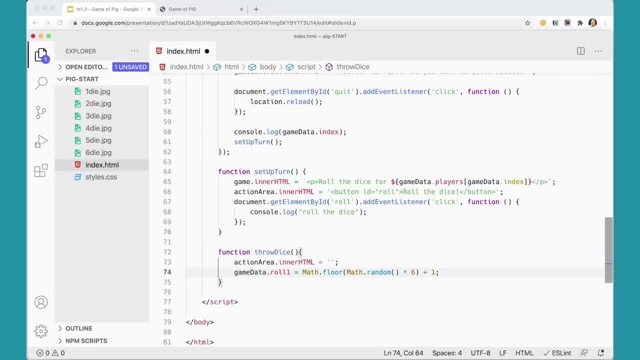 I could do math dot random times times five, right, And that would give me a zero to five, And then round it up using math dot sealing or math dot seal And round it up to you know, so that if it's. 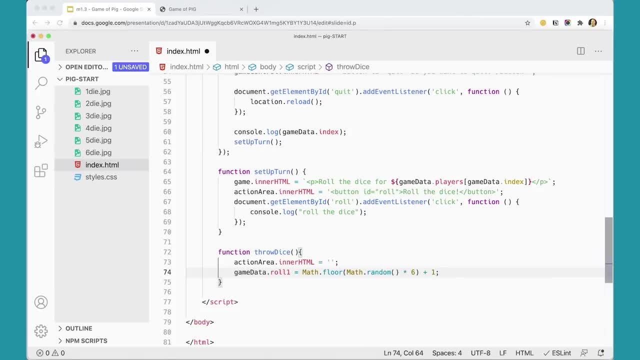 so it gets rounded up from zero to one, to one, to two, to two, to three and so on and so forth, If it's a partial number there. but there's a small, very small error that could happen with that. 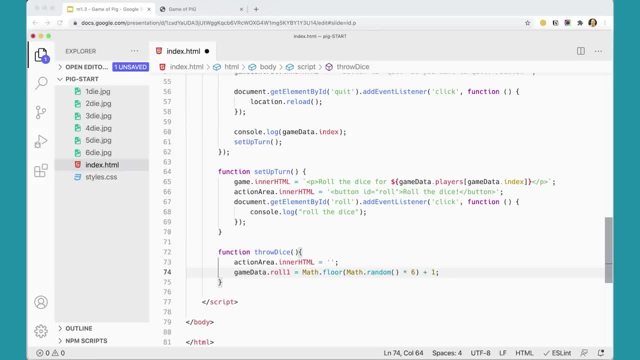 which is, if you remember, what math dot random does is it generates a number between zero and one, but it's zero inclusive. So it's very unlikely. It's very, very unlikely, but it's. it's possible that you could roll a 0.00000,. 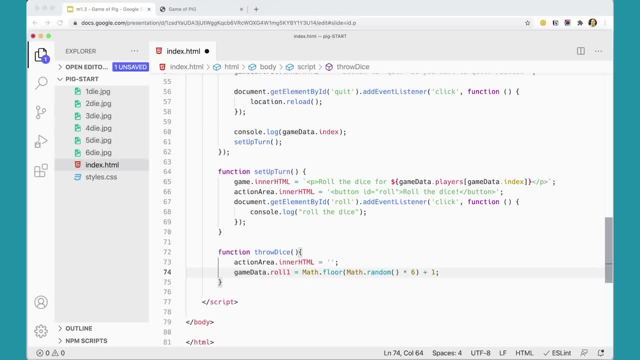 in which case math dot seal will not round that up to one. So you could potentially get a zero, a one, a two, a three, a four, a five or a six if you were to follow that methodology. And we don't want a zero. 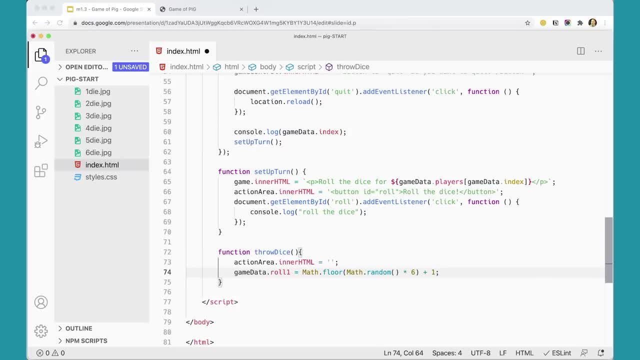 We want it always to be a one, two, three, four, five or six to match our numbers up there. So for our dice. So that's our roll one And roll two is exactly the same thing. We're going to generate a new random number for that. 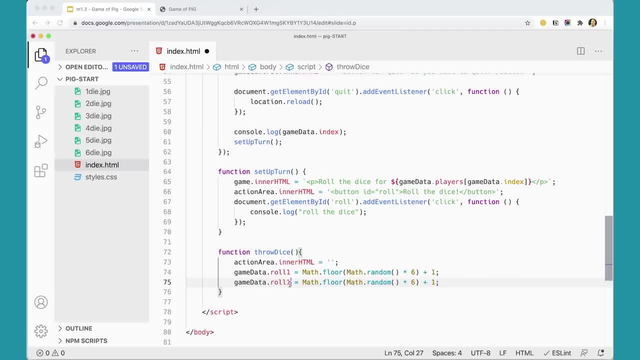 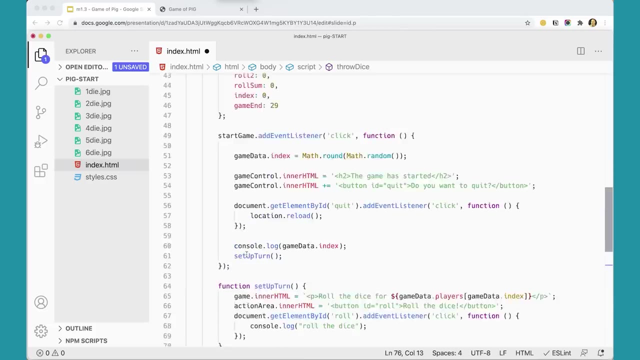 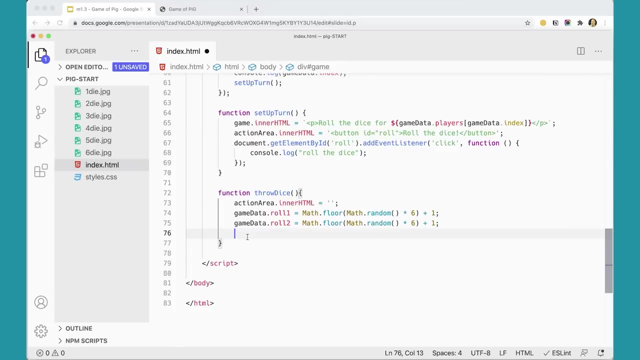 So roll two is also going to be the same thing. So we've got our two rolls there And then we need to set a message on our screen. We're going to put a message inside this game div here And that game div is going to say game dot- inner HTML. 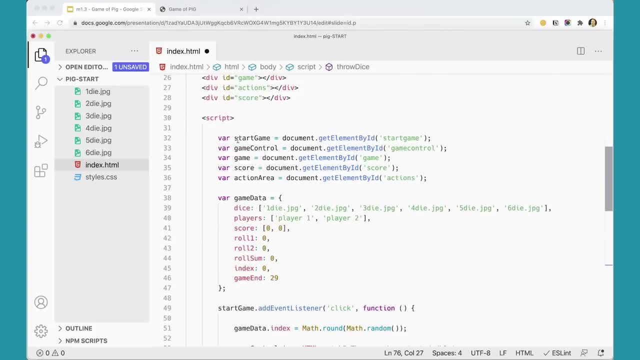 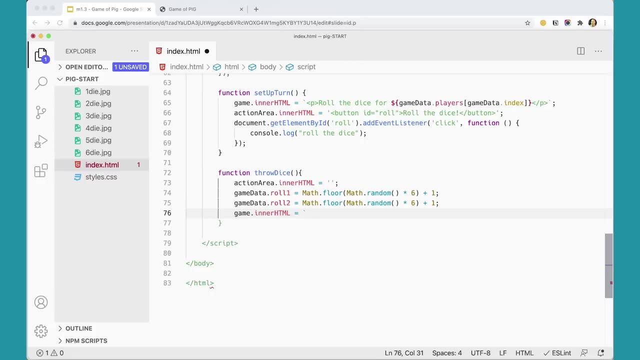 And we can just use game, because we defined this, this variable up here. That's going to go get that thing. Okay, Game dot. inner HTML equals, and I'm going to use my tick marks again because I'm going to use my variable in here. 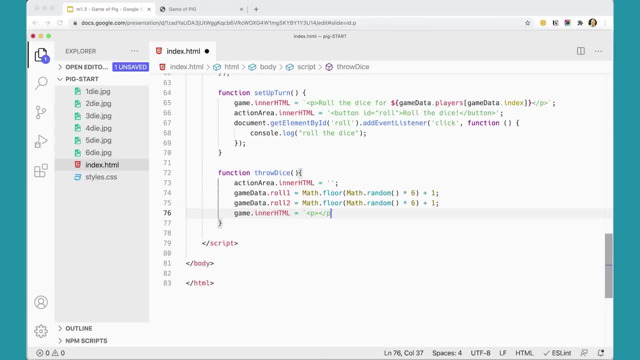 P. open and close the P. especially when you're working with HTML inside of tick marks like this, make sure you open and close it properly, because your code editor won't do the auto closing thing for you In the, in this case. 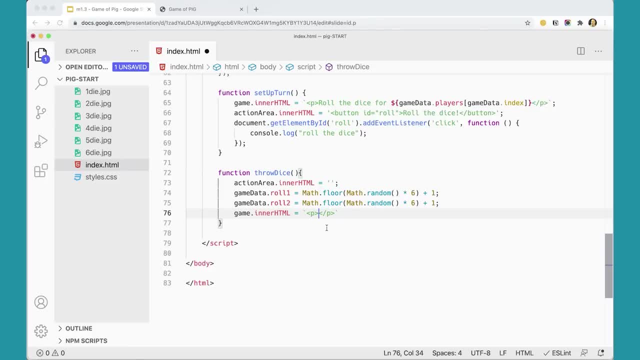 probably, unless you've got some plugin that does it. I don't know of any, but there might be some. Okay, Roll the dice for player X And again, player X is going to be a variable. Which variables are going to be? 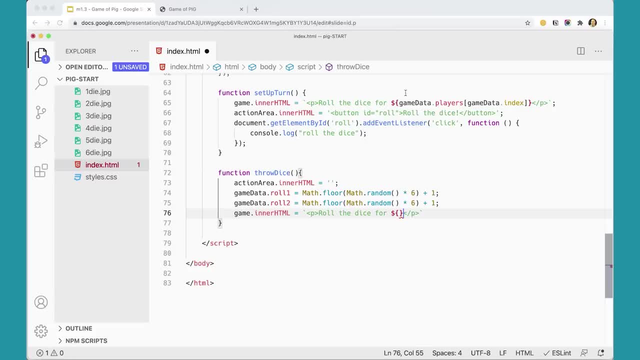 Dollar sign- curly braces. It's really just going to be this one again. We can even just copy and paste from here Game data players which, whichever player we're on it'll be played. This will be player one or player two here. 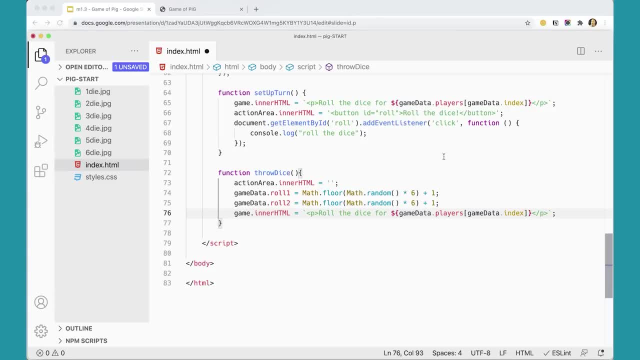 It gets put in there. Okay, great, Don't forget a semicolon. The next thing we need are the actual pictures of the, the two of each of the dice, pictures of the dice, And that's going to go inside the same div. 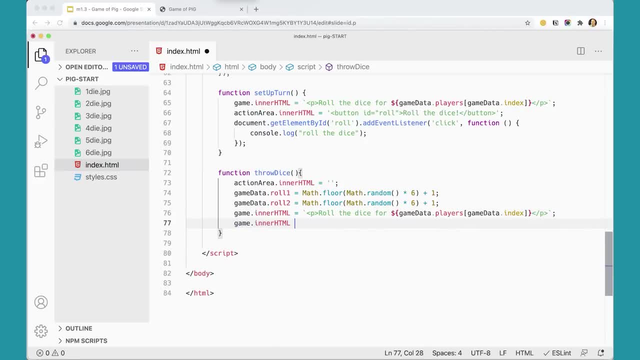 So I'm going to do game dot inner HTML plus equals to add to it, And again I'm going to use my tick marks, like so The semicolon, And in here I'm going to put in an image tag: IMG. 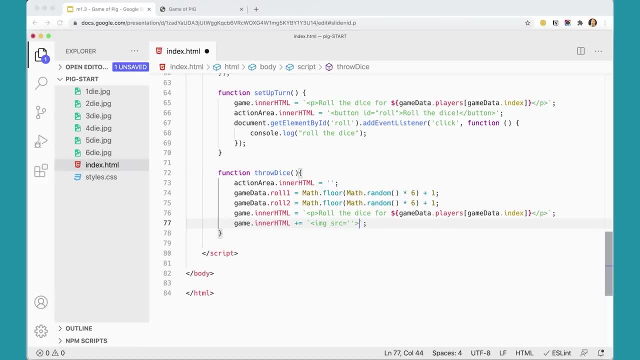 SRC equals quote, quote, like so That's going to be this. And then to get to one of my images, it would be, you know, something like die one, die two, die three. I don't know exactly what that is. 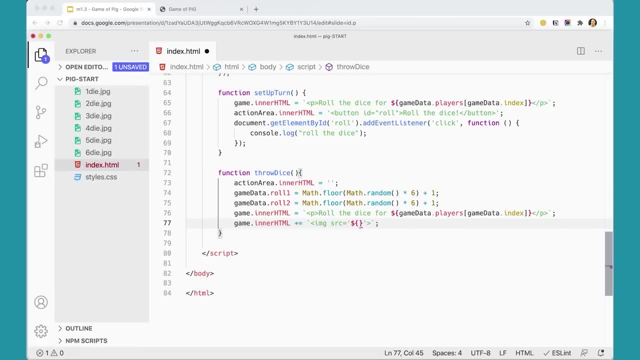 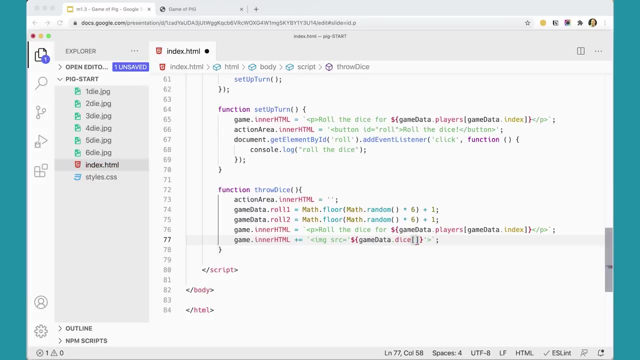 but it's really going to be a variable right? So it's going to be dollar sign, curly braces, Game data Dot. Which element do I want up here? I want my dice element, dot dice Square bracket. And which one do I want? 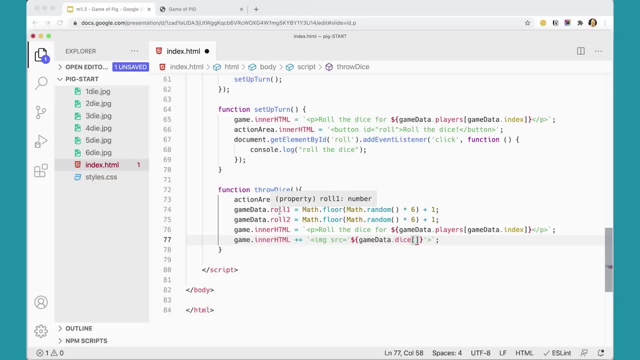 Well, it depends on what I rolled here for roll one. We've set roll one here, Game data Dot roll one, But I need to add one to it Plus. Actually, I need to subtract one from it, Minus one. 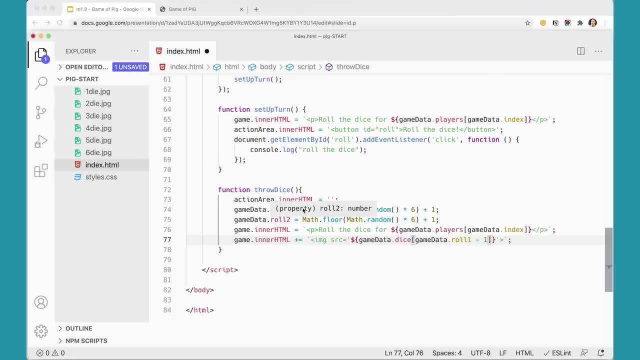 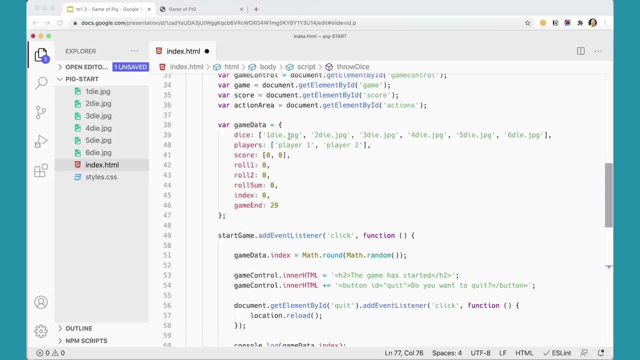 Because, remember, this is going to be a one, two, three, four, five or six. If I roll a one, I need element zero from this array up here, So I need to subtract one there. Game data: Roll one. 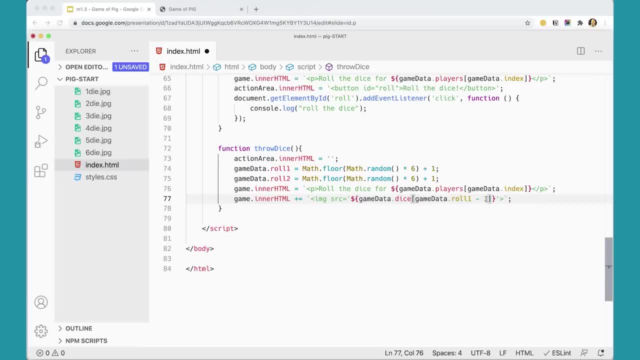 Minus one, I think I need to put. Yeah, I think that's right, Kind of prefer to have double quotes here, I think, Quote there, Double quotes And an extra one for me. There we go, All right. 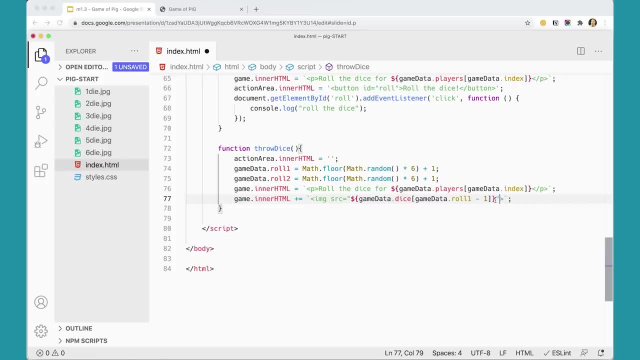 So that will put in our source, And really it would be good to have an alt attribute as well, For good. HTML equals quote Dice Die, Or I could even- You could even do this thing again if you wanted to. I'm just going to leave it like that. 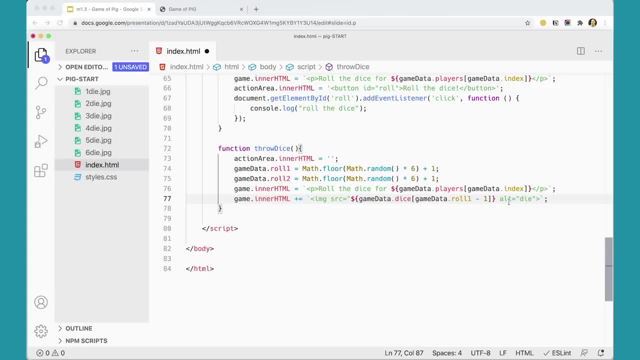 That's fine, All right. So we've added that image. That's the image for our first roll. We need an image for our second roll, which is going to look exactly like this, Except That this is now roll two, And then the last thing that we need to do is add up these two rolls together. 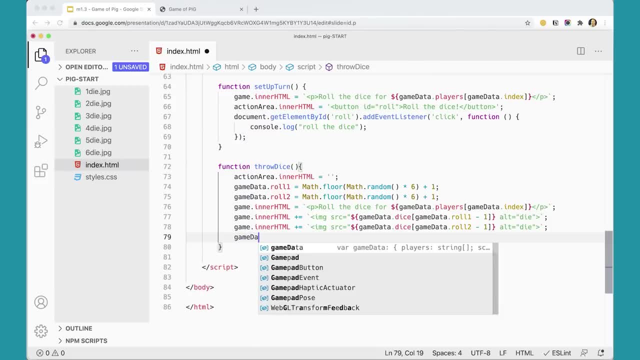 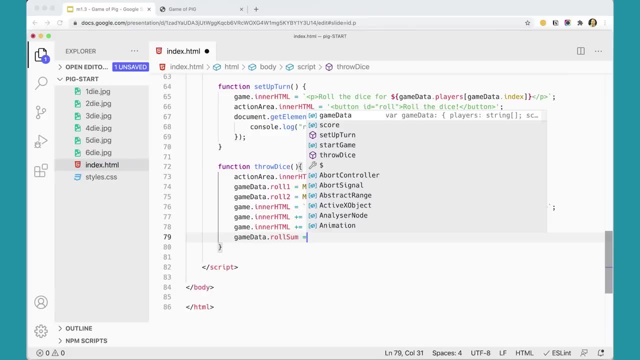 And put them in the sum total. So game data Dot Roll. sum That one there Is going to equal Roll Game data Dot Roll One Plus Game data Dot Roll two And that will add those up and put them in there. 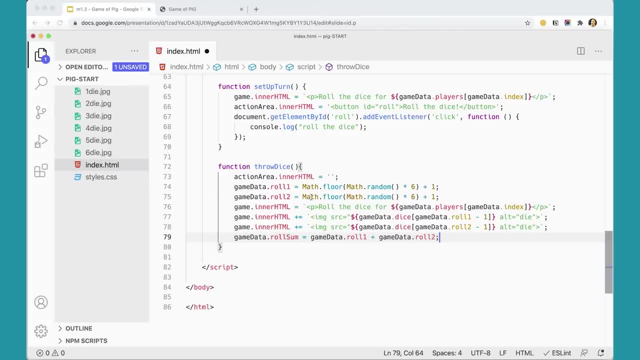 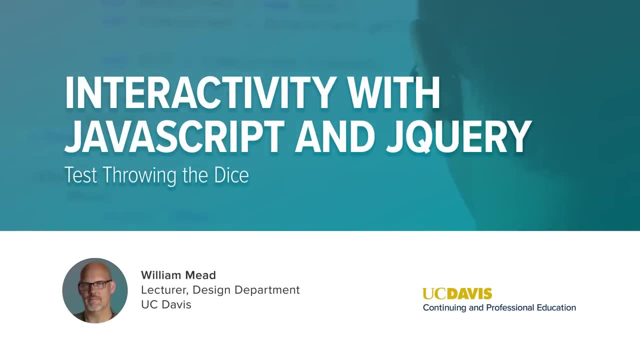 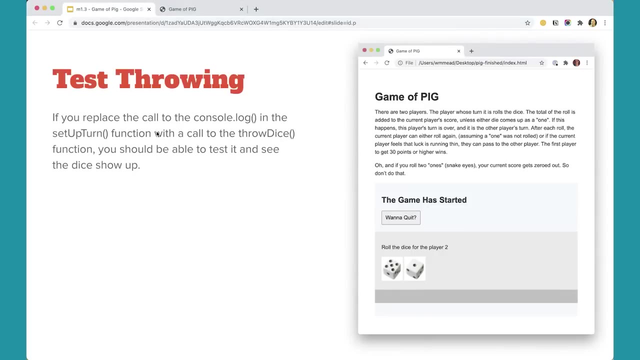 Okay, great, We're going to test this in the next video. You've started your dice throwing function, So let's test it and see if it works. All we really need to do to test it is replace the console log in the set up the turn function. 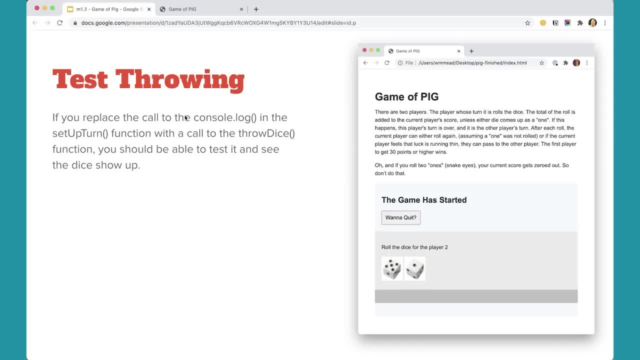 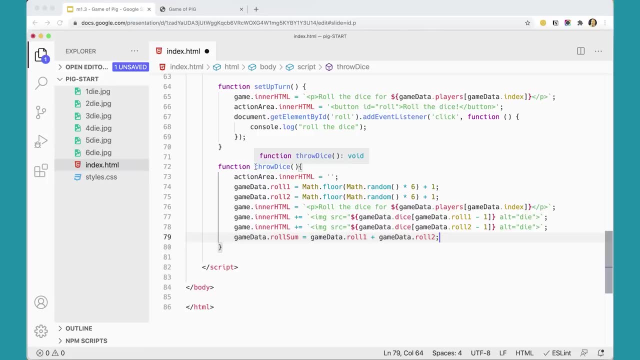 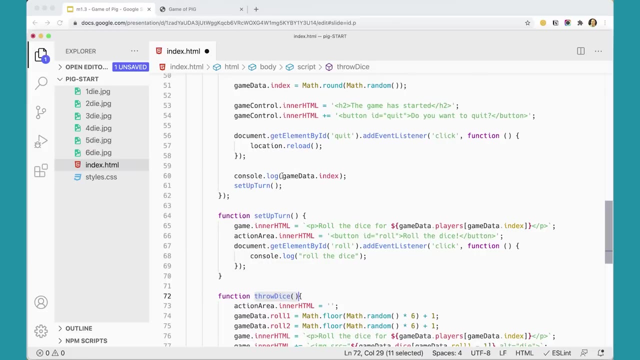 And replace it with the throw the dice function. So let's take a look and see how that works. So all I need is to take this function here and copy it And put it up here instead of. No, actually I didn't have a console log up here. 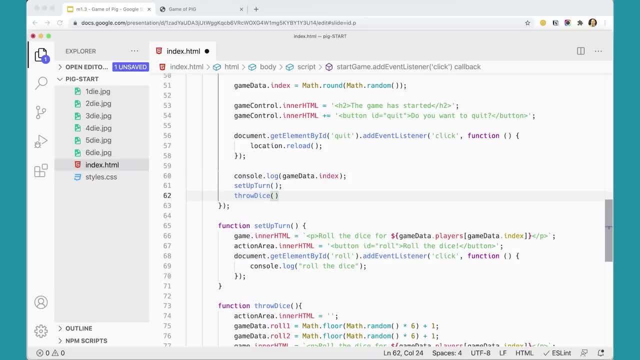 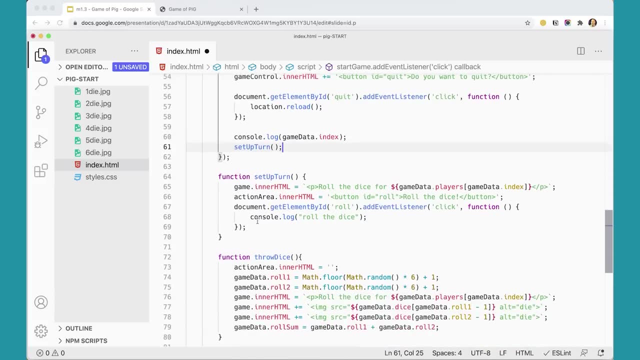 Let me just stick it in there. Throw the dice. Oh, I'm sorry. No, that's wrong. It doesn't go there. It goes here Instead of this console log: roll the dice. It goes here. Make sure you put it in the right place. 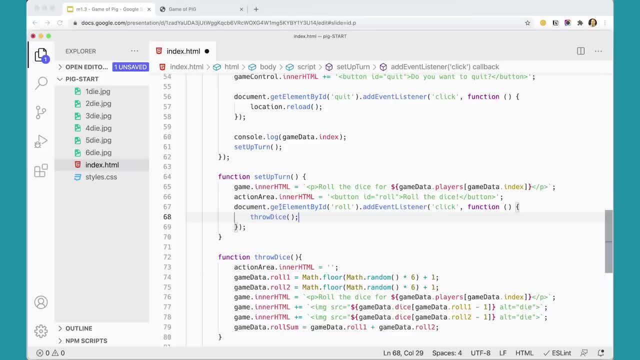 Don't make my mistake. Okay, So in the set up the turn function we throw the dice So that one starts set up the turn. set up the turn throws the dice once the turn has been set up And you click the roll the button thing there. 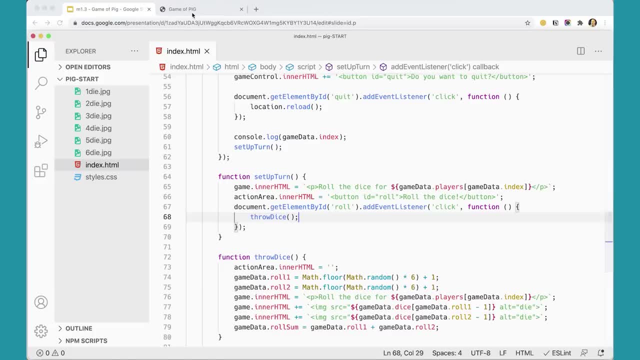 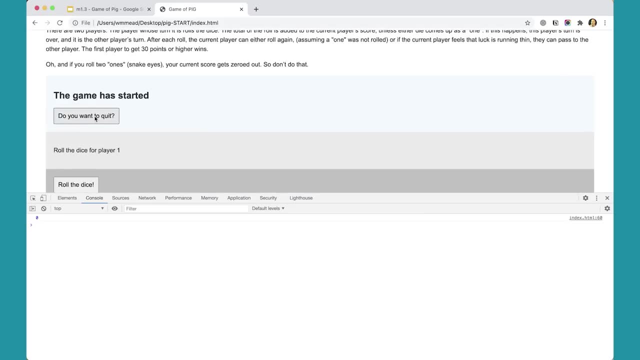 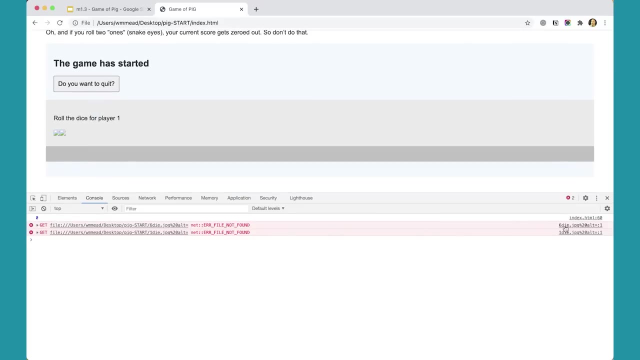 Okay, Let's see what that gives us. Let's save this and come over here and test it. Now, if I refresh and randomly pick a player, I can roll the dice. Whoops. Error file not found. Six diejpg alt. 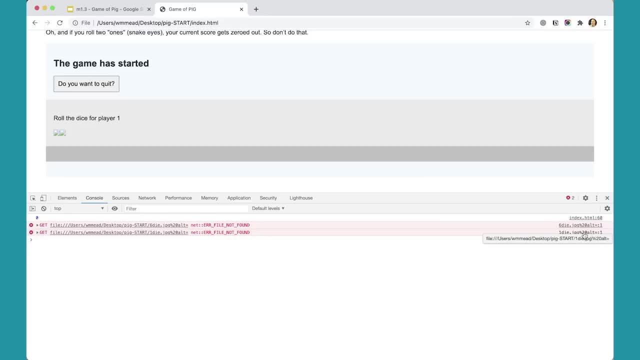 I can see right here that I forgot to close my. So this is very easy to have happen when you're working with HTML inside of a string, And I can see right here what's gone wrong. I can see that I forgot to close something. 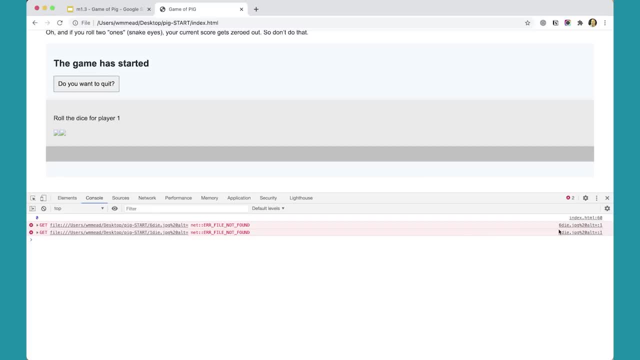 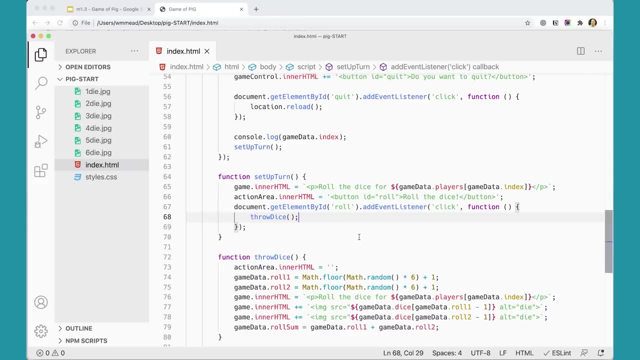 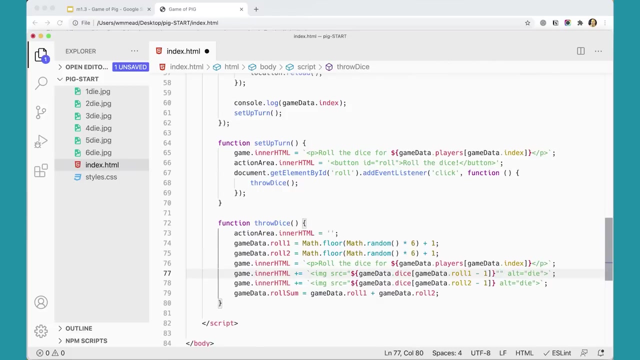 So it thinks that my whole image has this name on here, which is incorrect. So let's go back over here. It's in here. I forgot to put a quote here. One double quote. It'll add two, but we have to leave one in there. 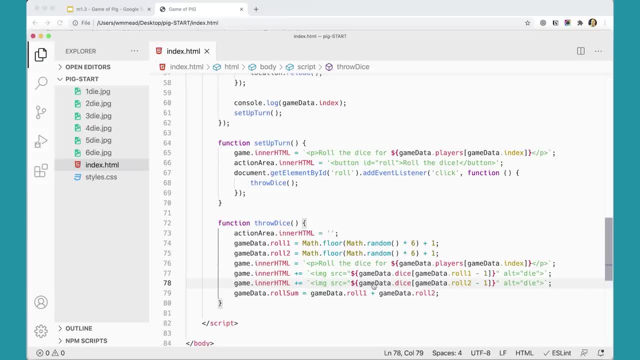 Okay, There we go, Save that. And this is normal. It's normal that while you're typing stuff, you're going to make mistakes. I make them all the time, Don't feel bad about it. Of course, I was trying to be fancy there by adding the alt attribute. 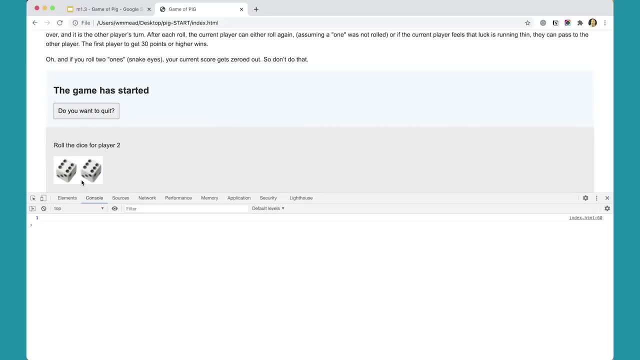 And really the alt attribute should be on there: Roll the dice. Now I've got two dice And it showed up And I can say: do you want to quit And start again? Roll the dice And I get two different dice. 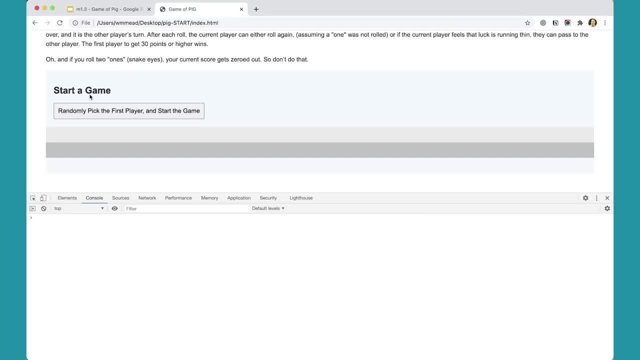 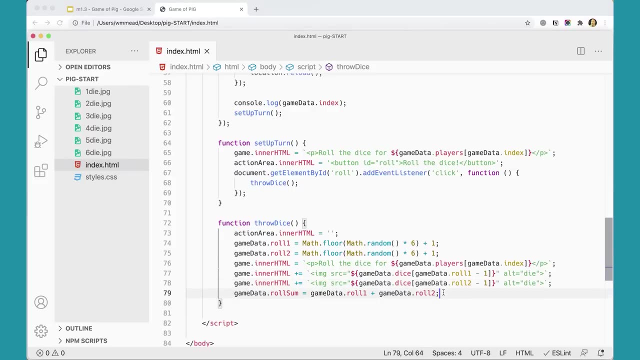 You have to refresh the page or click. do you want to quit each time to get this to work. And if you wanted to go even further, you could come in and add a console log And see what gamedatarollsum has in it. 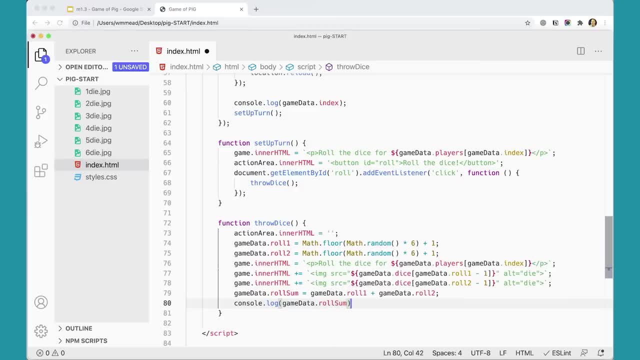 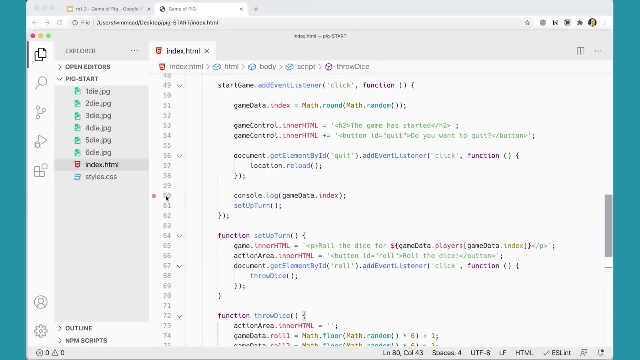 Or what any other variable in there has. if you're just curious to see what's in there, You can save that And up here. maybe I don't need this one anymore, The one that's giving you one or two. You can just comment it out or you can delete it. 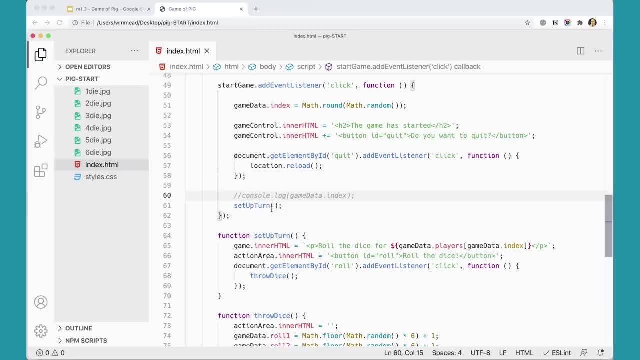 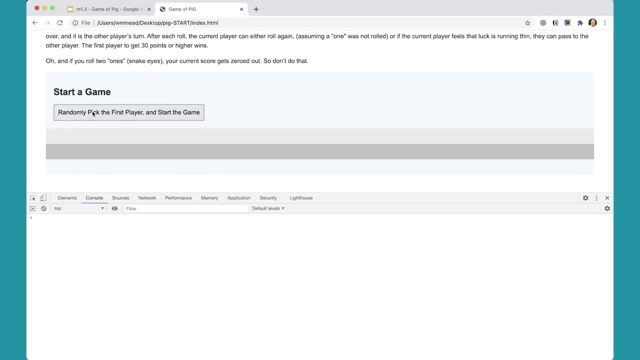 You can do whatever you want to it, But we don't need that one or two shenanigans anymore. All right, Let's go back and do that. try again. I'm going to refresh And I'm going to start the game. 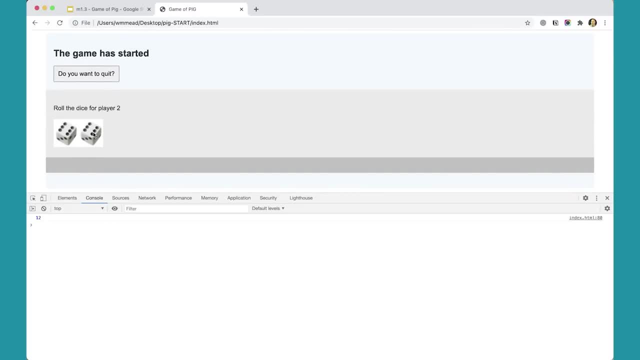 Roll the dice And you can see. I rolled two sixes- again That's something- And got 12.. Unfortunately, we're just going to have to click the button Or just click refresh, And here I got five And I'm going to press play. 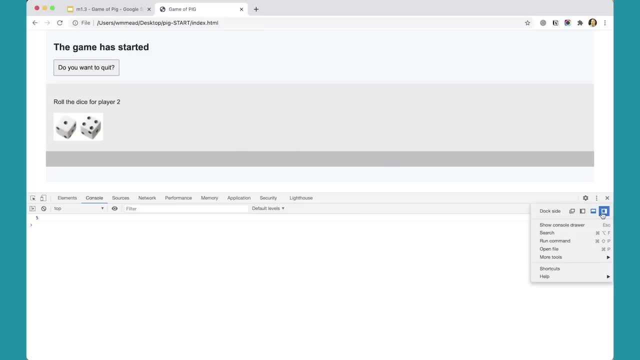 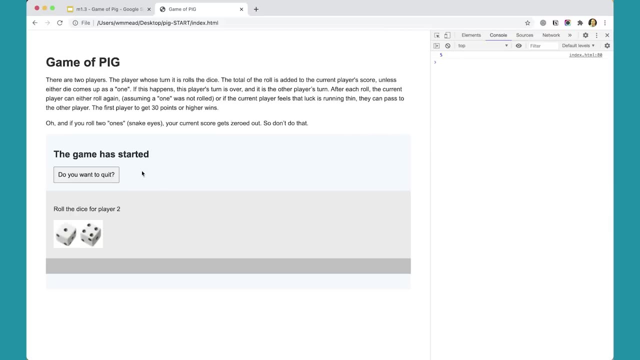 I'm going to move this inspector inside And we can do the same. It's going to move this over here. OK, So that's all working And I'm working really nicely. So now we have a dice game where we can throw the dice. 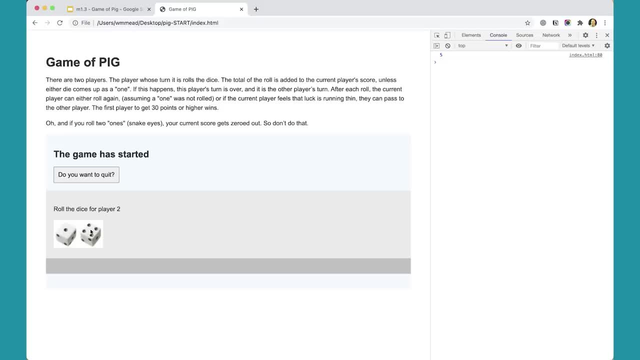 And the two dice will roll And one will roll each other. Those two will just, And that's fine. Now the next thing to do is to figure out. OK, What do we need to do? Do we need an ipsy? 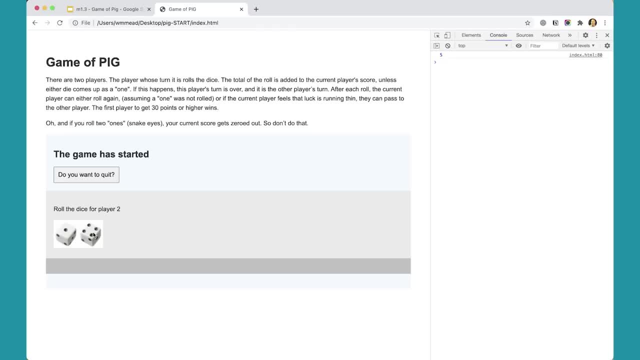 Do we need some sort of ipsy? OK, If two ones. In other words, if the roll sign is ipsy, then we. If one of these, And this is ipsy, If one of these, And then we can. 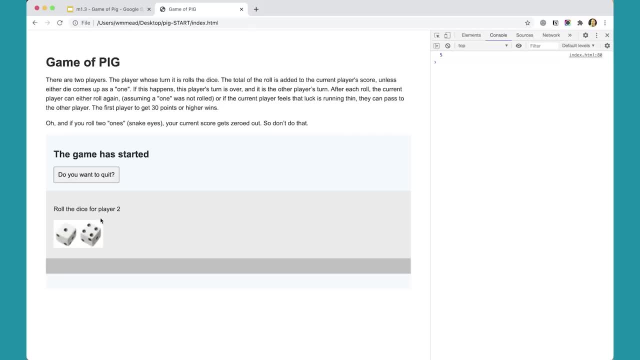 And then we can, And then, And then roll the dice Down here And then we can put out the ipsy. This is going to be very easy. We're going to actually write the ipsy And the die out, Because in the game if we have an ipsy, then we have a die out. 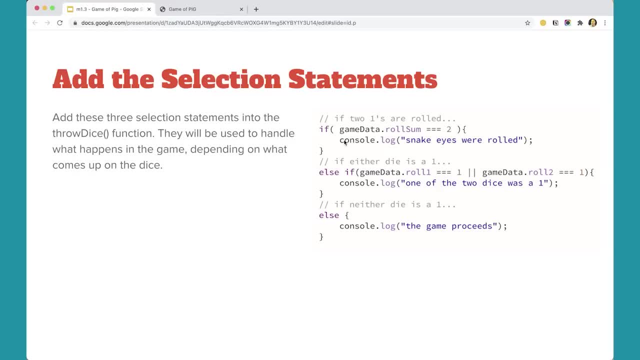 So, for example, ipsy and then the die out. You have a die out, And then we have ipsy And the die out will be ipsy. And then we have ipsy, And then you have ipsy And now we have a die out. 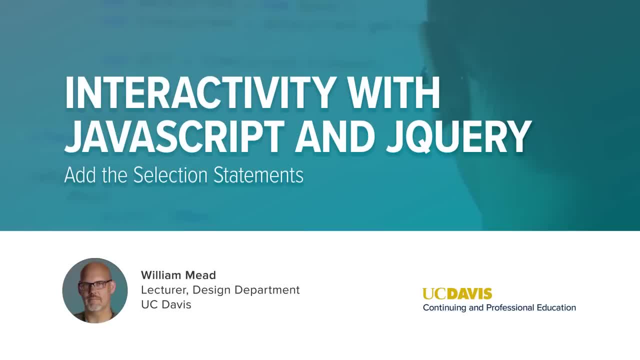 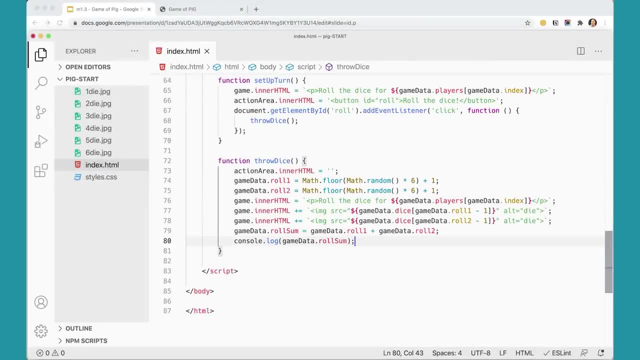 And then you have ipsy, And then you have. We're going to add if statements into our throwDice function here. So if- and the first one is if, gamedatarollSum is the same as, exactly the same as a 2.. 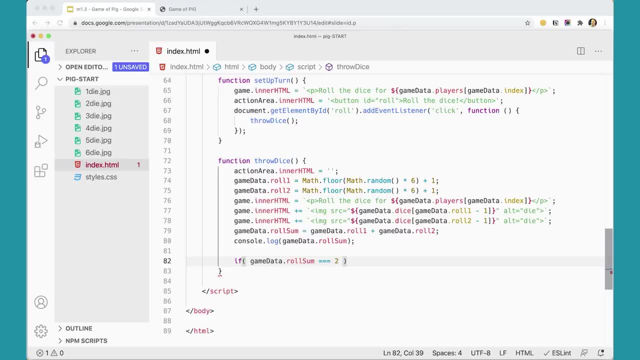 The only way you get a 2 is if you've rolled two 1s. If it's exactly the same as a 2, then we're going to say something like consolelog. We'll fill this out later with more specific instructions, but for right now I just want. 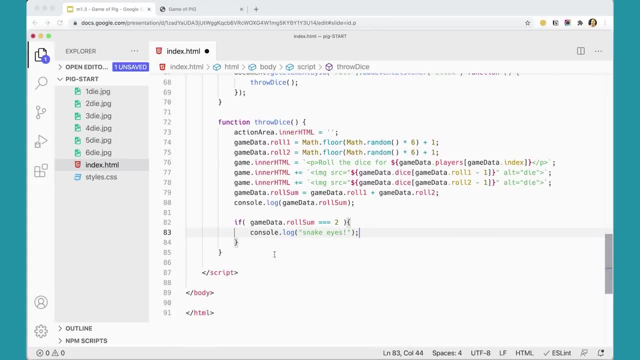 to know. I just want to capture that situation. And then we've got an elseif And we want to check two values. We want to check the value of roll1 and the value of roll2.. And if either one of them comes up a 1, we want to do something. 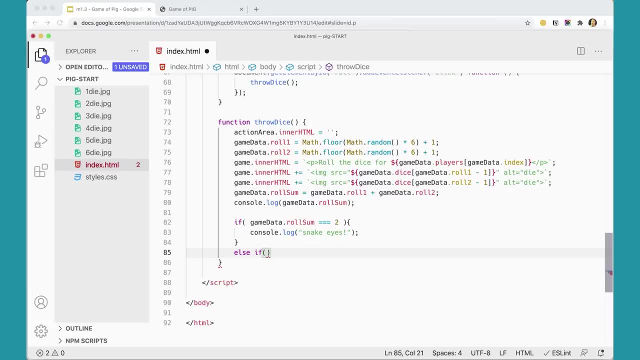 So that will come back true if either one of them is a 1.. So the way to do that is to say, if gamedataroll1. Is the same as 1. Or there's two pipes, gamedataroll2 is the same as 1.. 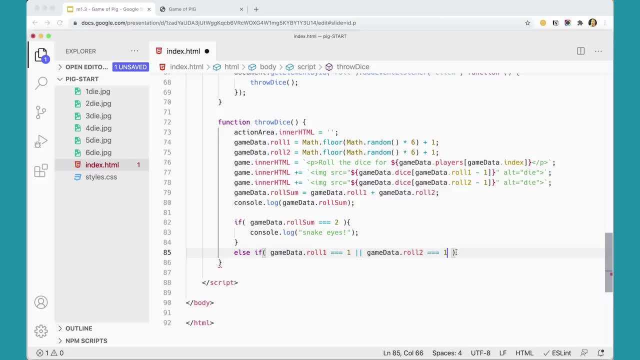 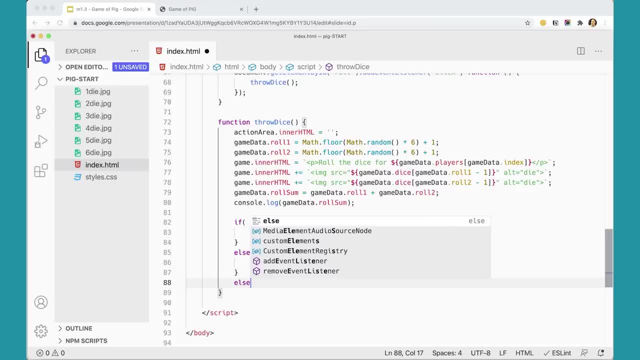 And then we're going to say, if that situation occurs, then consolelog. And then we're going to say, if that situation occurs, then consolelog, And then we've got the else, And then we've got the else, And then we've got the else. 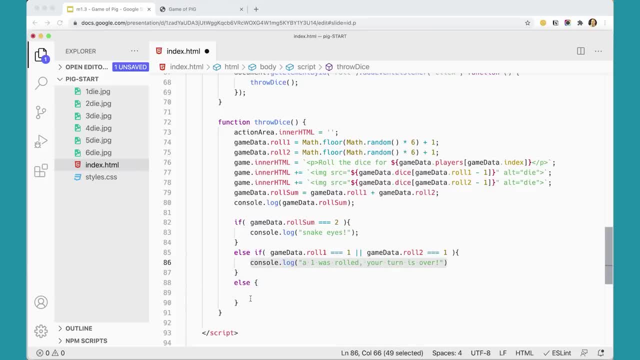 And for that we can just copy this, paste it and say: the game continues, Roll again or pass, And we'll deal with that separate. So now we've got three situations. So now we've got three situations. So now we've got three situations. 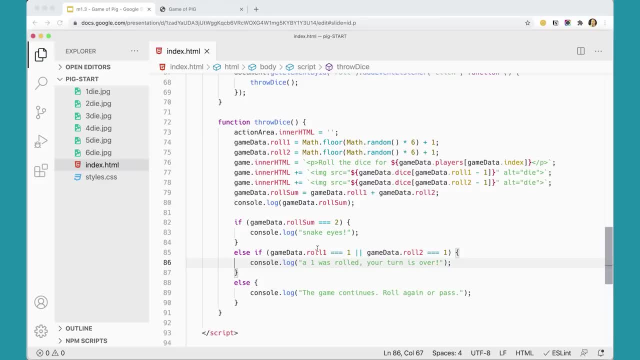 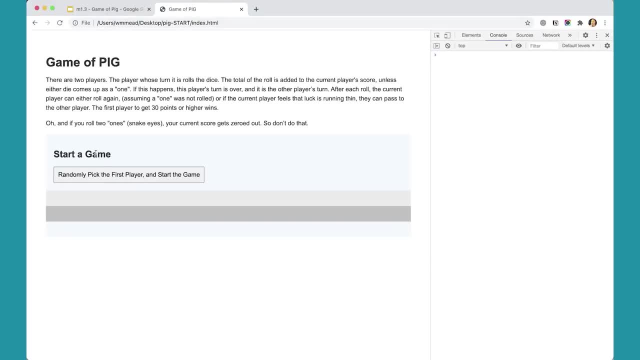 And come back here and refresh this. Pick my player, Roll the dice. I got an eight. The game continues. Roll again or pass. I got two fives. The game continues: Roll again or pass. I'm not getting anything. 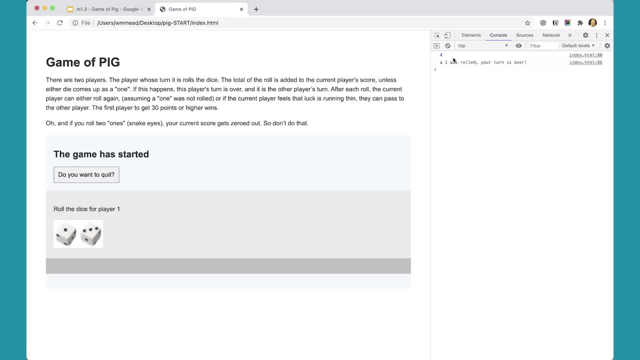 I'm not getting anything. Okay, here I got a one. The one was rolled. Your turn is over. Not lucky enough to get Snake Eyes to test that, But you can keep going along and seeing that these numbers add up correctly and that it's doing the right thing until you've gotten all of those things checked. 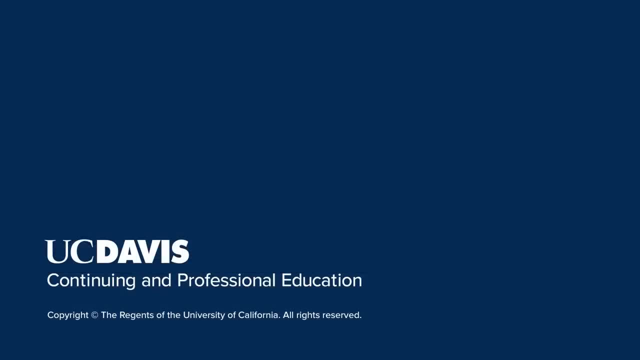 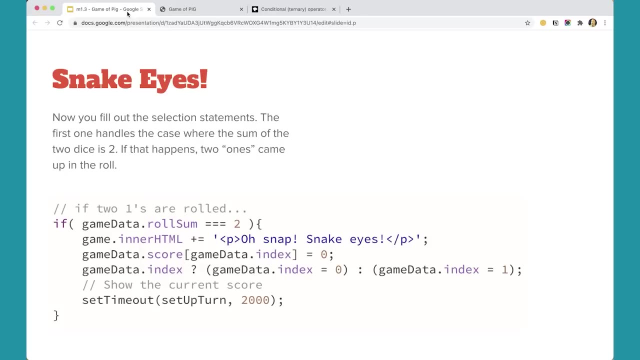 Let's handle Snake Eyes first. So we'll fill out each of these if statements, but we'll do Snake Eyes first. So if we get a two, let's deal with that. First thing we're going to do is add to the inner HTML of the game and say something that tells us that we got Snake Eyes. 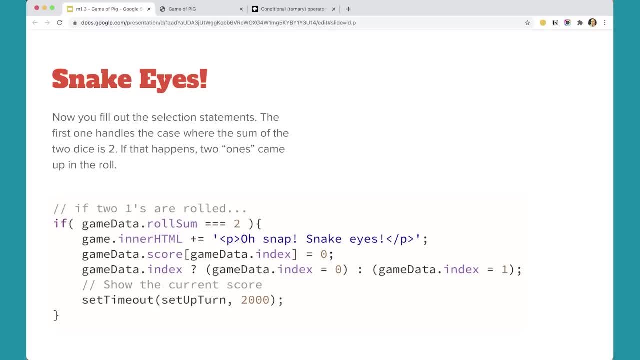 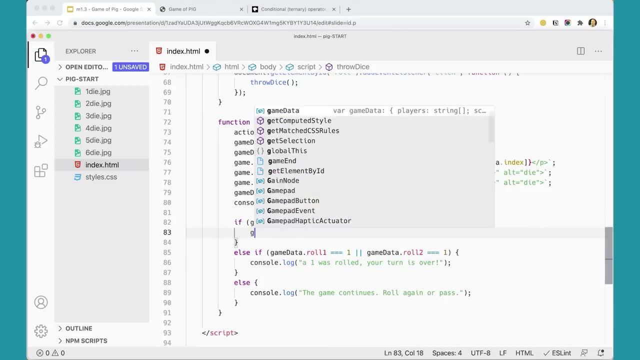 So let's do that, so we can alert the player that they got Snake Eyes. So in here, Game, Game, Game, Game Game gameinnerHTML plus, equals, Plus, equals, because we're going to add to it and something like: 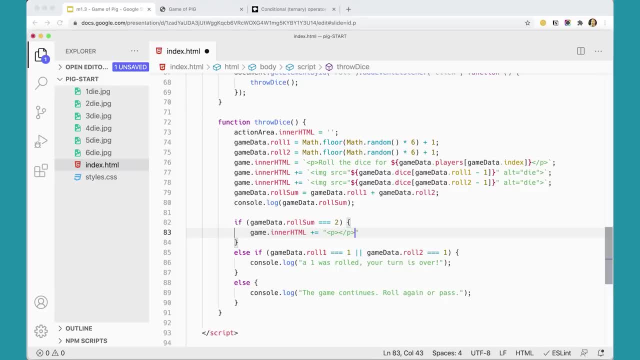 Oh snap, Let's close the paragraph first. Good practice there. Oh snap, You got Snake Eyes, Something like that, So that's going to just put a paragraph in there. that has that. The next thing that happens is that the score for that player gets zeroed out. 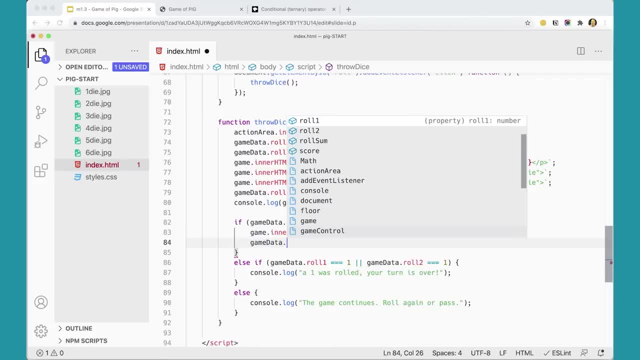 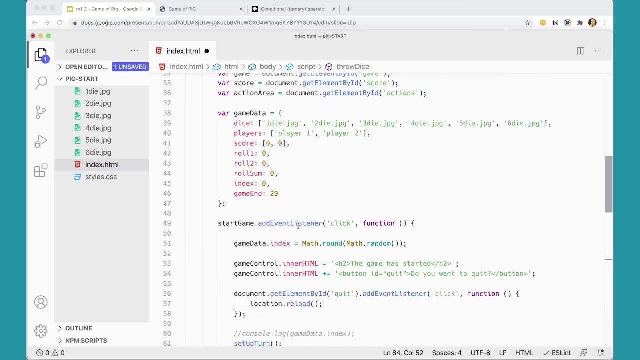 So gamedatascore is going to be set to zero. We set that back to zero. gamedatascore is going to be set to zero. We set that back to zero. So that means we're going up into this gamedata, finding the score for whichever player it is. 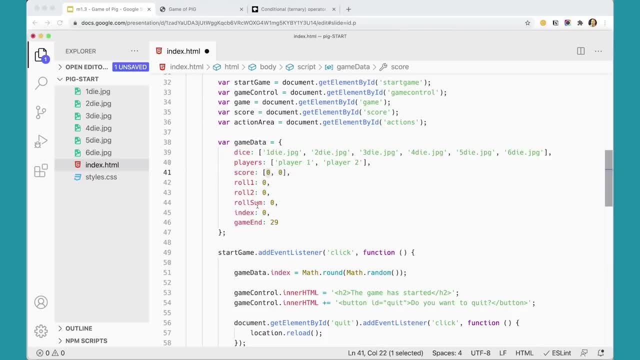 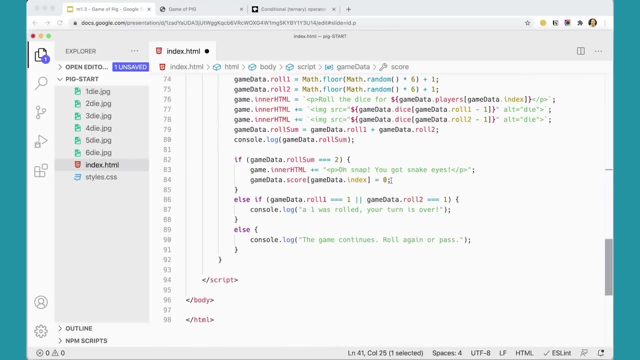 If index is zero, we'll set this one to zero. If index is one, we'll set this one to zero. So we're setting it to zero there because we're zeroing out their score, because that's what happens if you roll two ones. 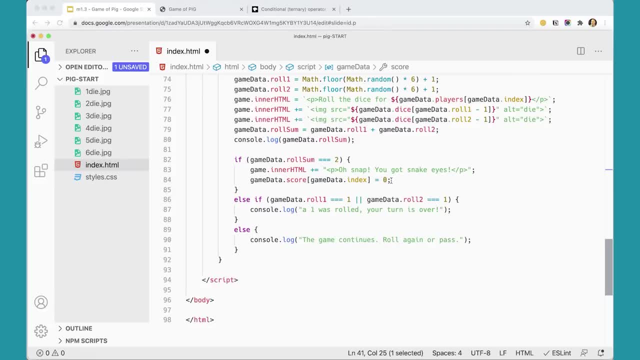 You lose all the points you've gotten so far. Then we need to switch players And we could do this with an if statement. If index is zero, set it to one. If it's one, set it to zero. We could do an if-else statement there. 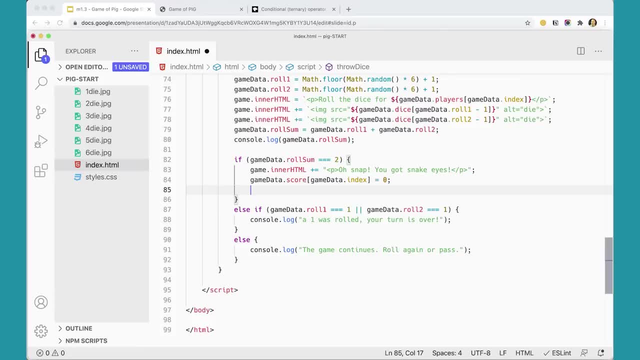 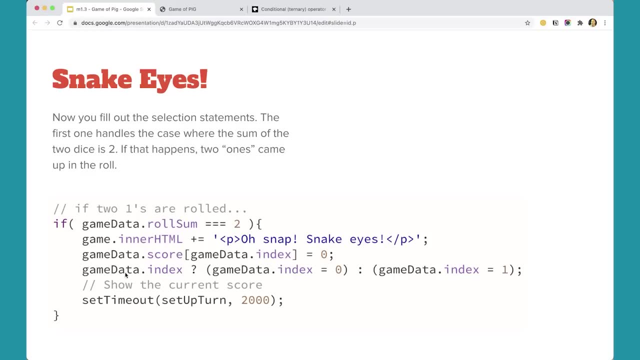 But there's kind of a nice shortcut way of doing that, And that's using what's called the ternary operator. We see it over here, So I'm going to set gamedataindex. So what happens here in a ternary operator is we evaluate whether or not this is true gamedataindex. 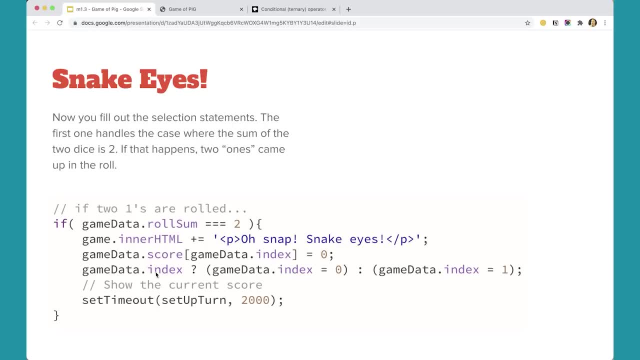 And remember, in general, we're going to set it to zero. In JavaScript, zero is false And the gamedataindex is either going to be zero or one. So if it's zero, then it's false, in which case we'll set it to one. 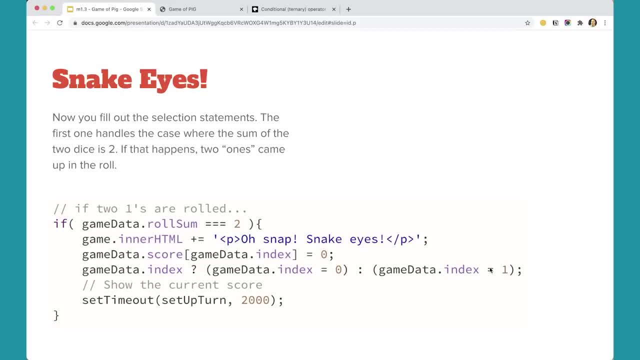 If index is true, if it's set to one, then it's true, in which case we'll set it to zero. So this is kind of a nice one-line way of doing an if-else when you're choosing between two things. 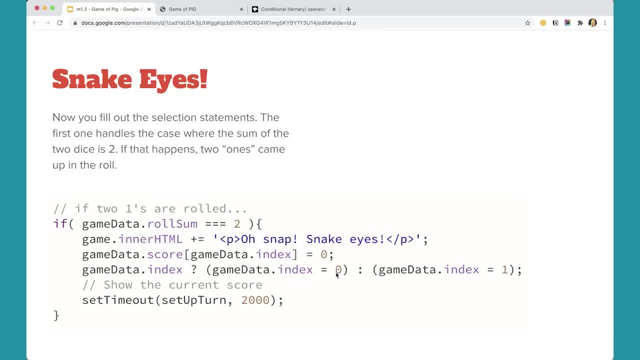 You can only choose between Two things. If we had three players, this wouldn't work, because we'd have to do some if-else statements for that. But with two players we can just say: it's either a zero or a one. 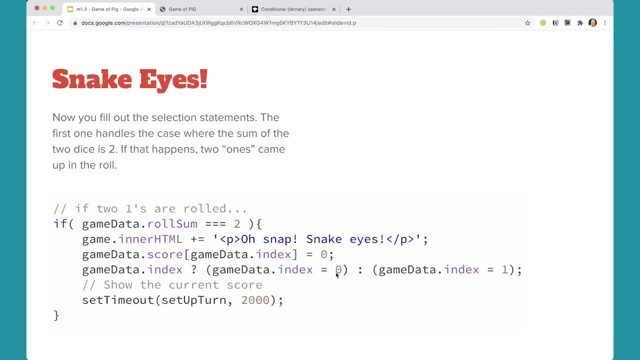 If it's a one, change it to zero. If it's a zero, change it to one, like that. So it's kind of a nice one-line way of doing this, And our function's getting quite long, so anything we can do to shorten it up is kind of nice. 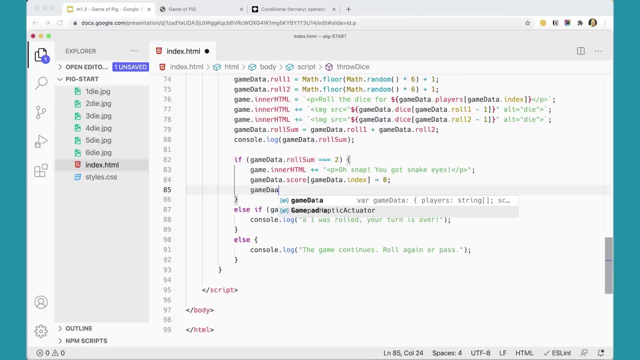 So gamedataindex, And then in parentheses I'm going to put gamedataindex equals zero, Because if this is true I want to set it to zero Or we use a colon here. So gamedataindex equals one. 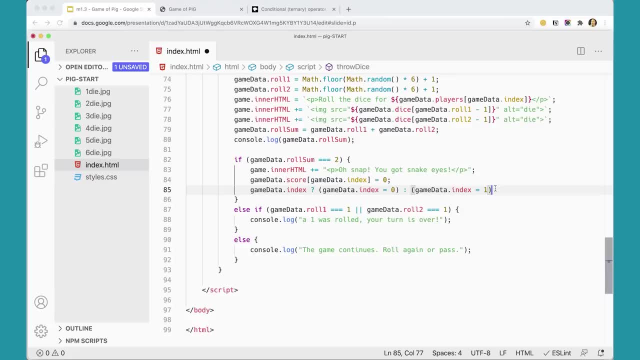 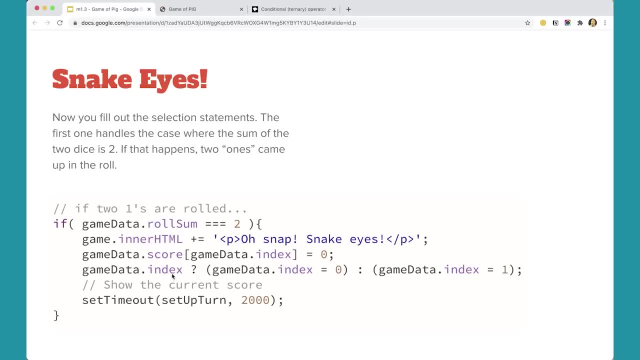 Because if it's false, if that's a zero, I want to set it to one. Hopefully I did that right. Let me just go check real quick over here. gamedataindex, question mark: Yep looks right: Zero and one. 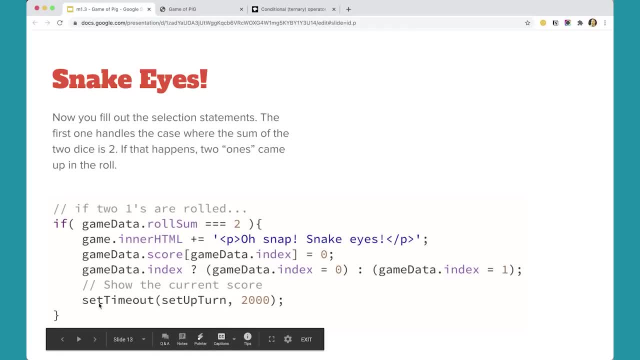 And then what we're going to do is we're going to wait A couple of seconds, Because we want this. oh, snap, snake eyes is rolled on the screen for a minute, Or not a whole minute, but a few seconds. 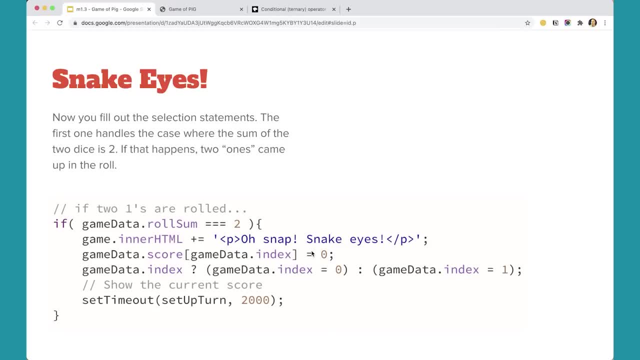 So that whoever is playing the game can actually see it appear. So I'm going to use setTimeout to just wait two seconds before I run setupTurn again. Run the setupTurn function again, Which will put us back with the correct player. So let's go ahead. 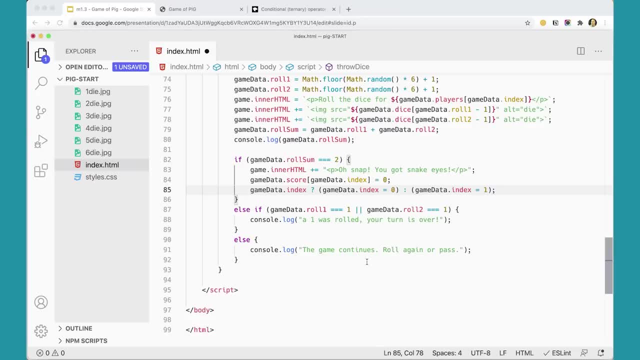 And add that setTimeout there. setTimeout, setupTurn after two seconds, 2,000 milliseconds, And that should work. Now, if we wanted to sort of test this before we go forward, it might be a good idea to do that. What we can do is we could just come in here. 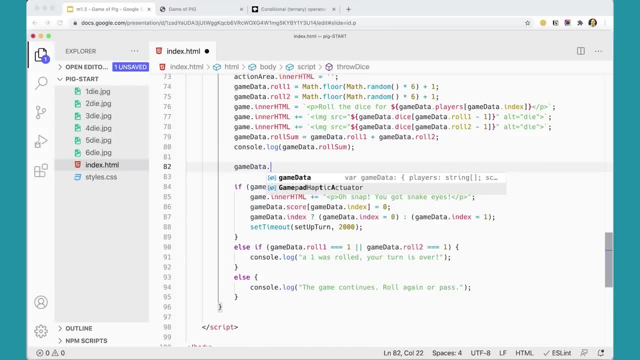 And just temporarily set gameDataRollSum equal to two. So no matter what we roll in this roll up here, this thing's going to get set back down to two And then this thing should run and change my player. Wait two seconds and set up the turn. 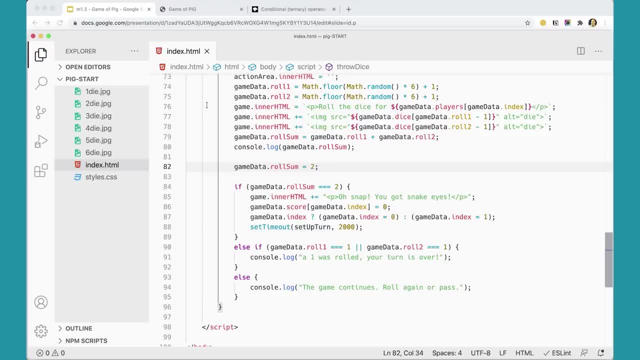 That way we don't have to sort of keep playing and rolling until we try to get two ones to pop up randomly In order to test this. So let's throw that in there and see what happens here. I come over here and test this. 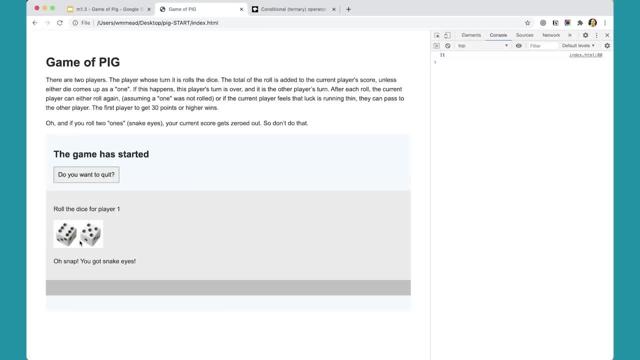 I can run my first player Roll the dice. It comes up with 11.. But then it waits two seconds and it says roll the dice for player two. Let's try that again. Roll the dice for player two. I roll the dice. 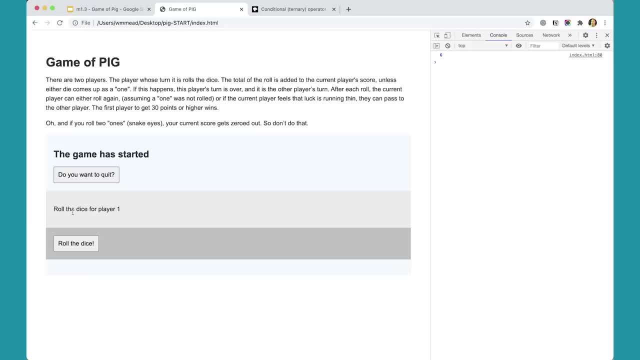 I actually got a one that time, But it switched it to two And now it says roll the dice for player one. So you can see that it's working, see that it's actually changing the changing the player, waiting two seconds and changing the player. 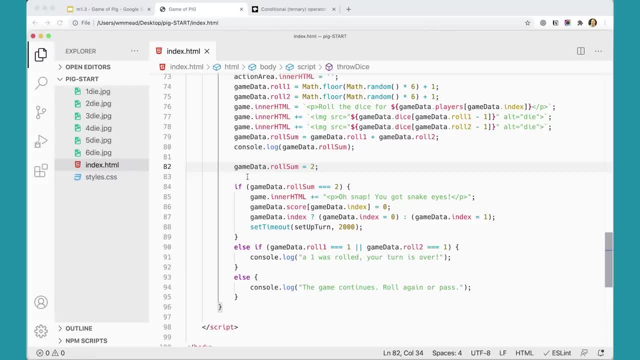 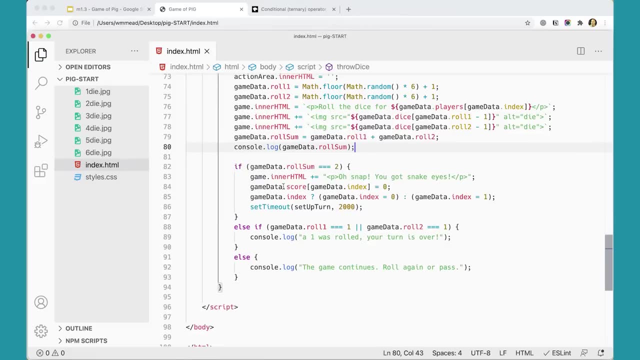 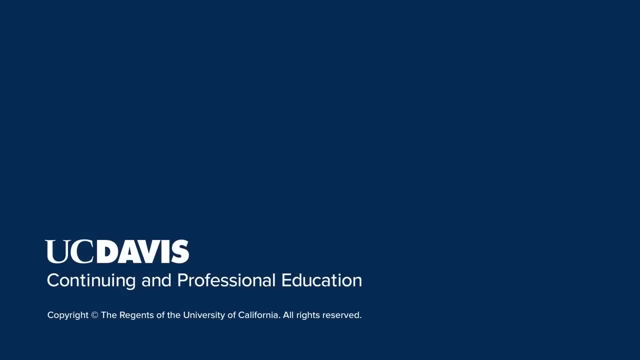 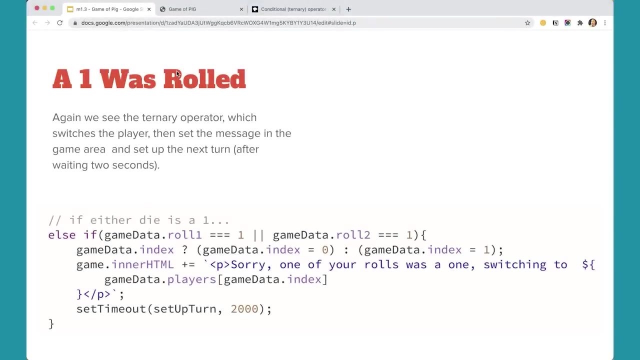 so that's actually working, which is great, so i can come in here. this is going to really mess things up if i leave this here, so i'm going to take that out and save that, and we'll continue in the next video. the next thing we're going to look at is if a one has been rolled, and, to start with, we're going to 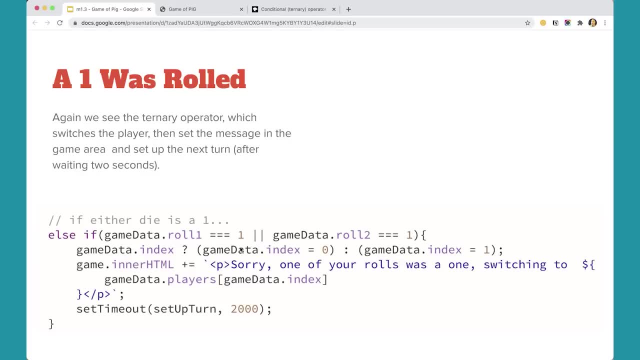 swap the players right off the bat. if anyone was rolled either of the two dice comes up a one, then we're going to swap the player. so let's do that first, because that's just using the operator again. so Let's come back here and get this ternary operator here. 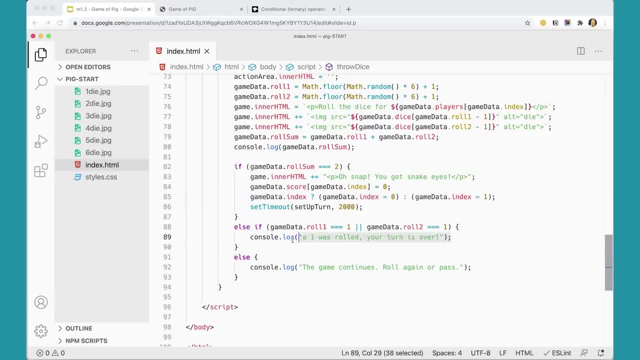 you can just copy and paste it and stick it down here and place it in that console log. and again, what that does is it sees what the value of index is and it determines if this statement comes back true or not. remember, index is either going to be a zero or a one. 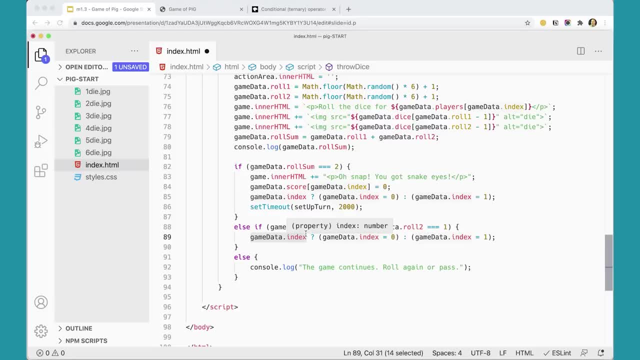 if it's a zero, it's false. if it's a one, it's true because, remember, truthy and falsy in general is not basically in javascript. so a zero in javascript is falsy. so if it's false, then it's going to do this, it's going to switch it to one. if it's true, then it's going to switch it to a zero. so, um and 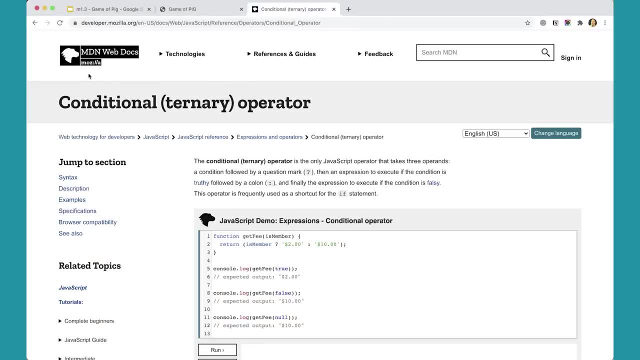 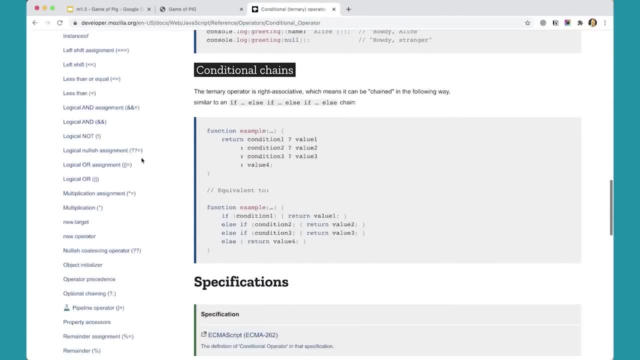 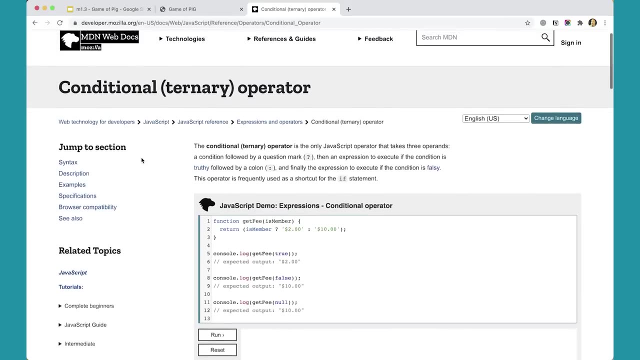 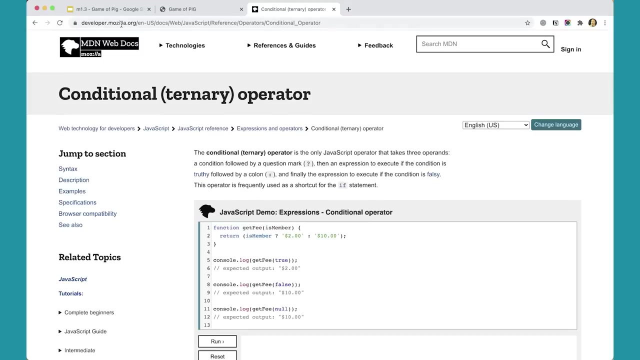 again up here i have a page loaded from the mdn web docs that will talk more about the ternary operator. so if you're more curious about this particular expression in javascript or this operator in javascript it's, it's worth taking a look at this page here. okay, so we've got. 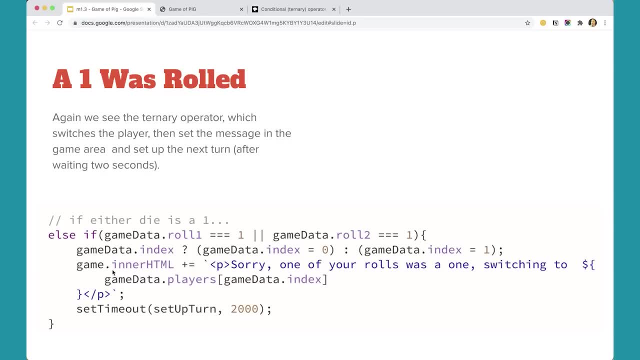 that the next thing we need to do is just set the game index. we're going to add to that. instead of adding, oh, you rolled snake eyes, we're going to say: sorry, one of your roles was a one switching to the other player, so let's go ahead and put that thing in there, and then we'll set up the turning. 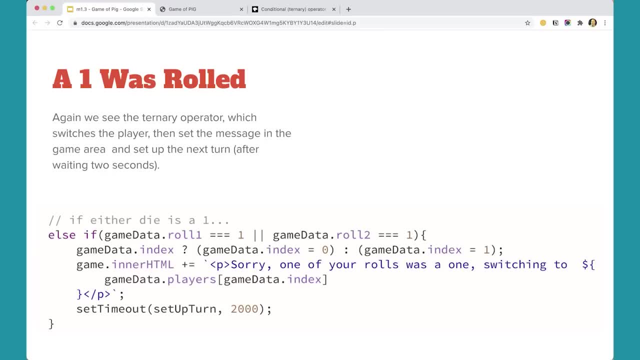 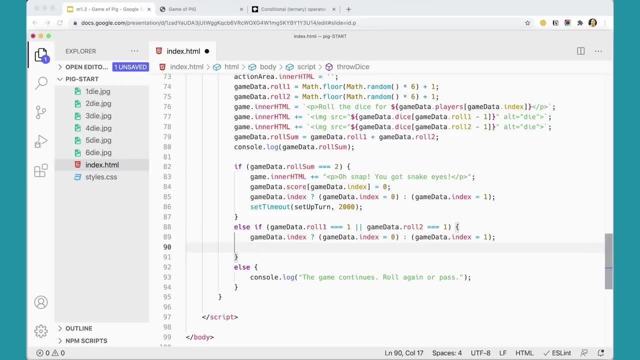 it and, and that's basically all we need for this lsif here. so in here, game dot inner html plus equals, and we're going to use our, our tick marks again in the semicolon. and in here we're going to add a paragraph p and and. 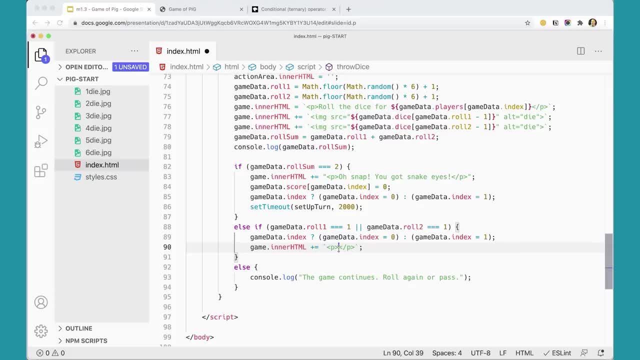 you rolled a one switching to the to other player, and really other player is going to be a variable dollar sign, curly braces, and really what we want is this reason why we wanted to do this line first, because we just switched that index if we were on player one. now the index is set to the other player, so this will just. 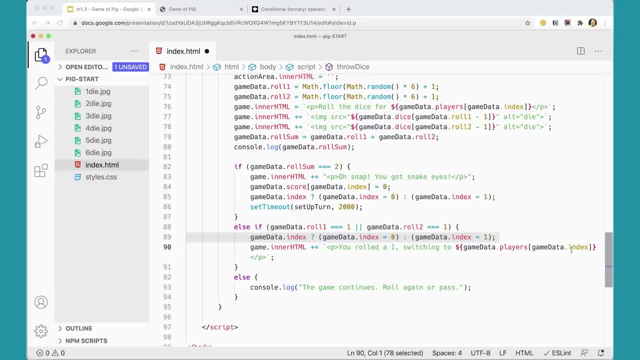 say play. you know, if we were on player one, this will just say player two. if we were on player two here, this will say player one. so that kind of goes back and forth and then down here. we just need to set time out and run, setup, turn again, and that will work. that should work just fine. 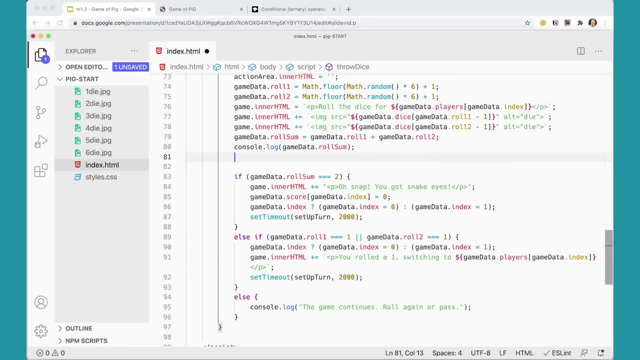 and again. we can test it up here by forcing one of these roles- game data dot, role one. i'm going to set that equal to one, just to test it. it's not, it's it's not perfect, but just i just want to see it without having to. 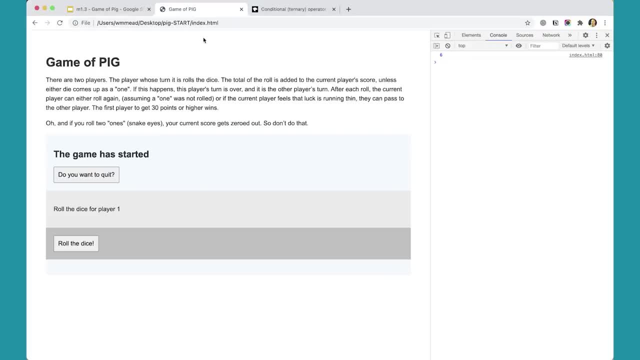 roll a bunch of times until i get a one, although that certainly comes up more frequently than two ones. let's refresh this. roll the dice for player one. you rolled a one, i didn't roll a one, but because we set it to say one of those dies is going to be one, it's doing it automatically. 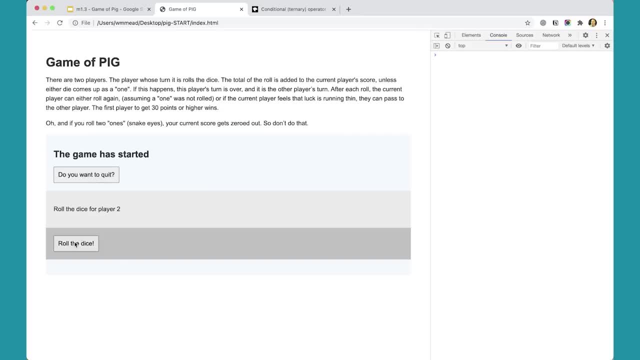 you roll the dice for player two, you roll the one switching to player one. and now roll the dice for player one. roll the dice, you roll the one switching for player two. roll the dice, you roll the one switching for player one. so you can see it's switching back and forth now and and working. 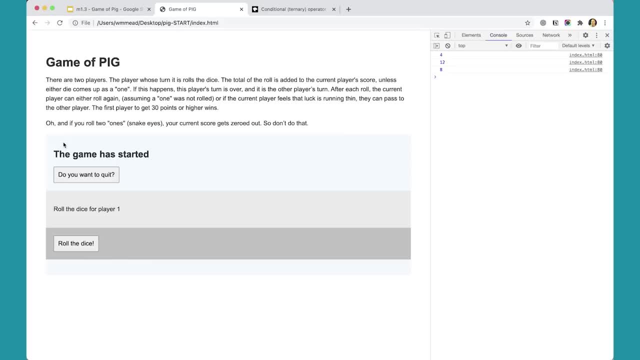 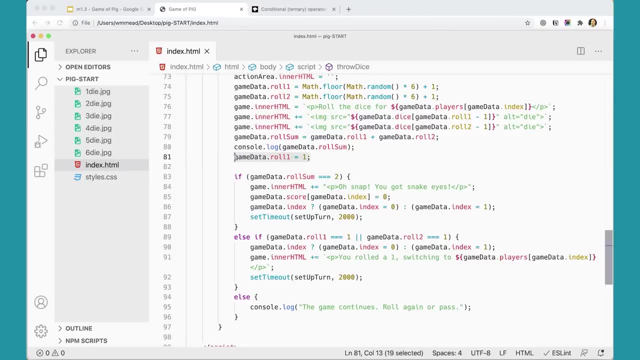 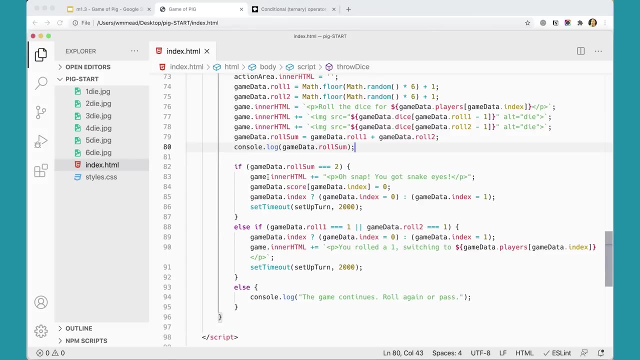 perfectly every time. so that's exactly what we want there. so we want to come back and remove this from here, because that will really screw things up later if we forget to do that. okay, great, so we've gotten both the situations for what happens if you roll two ones or if you. 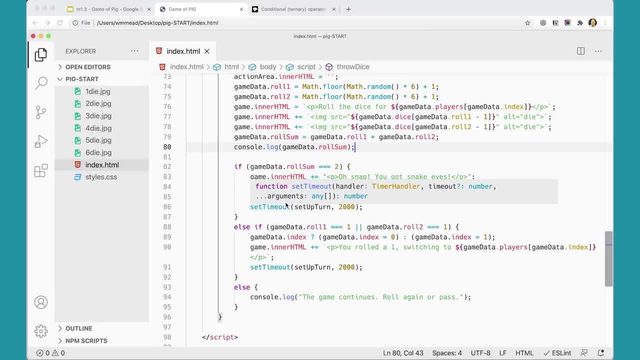 roll, or if either of the dice come up, a one. we've gotten those sussed out. next we need to figure out the else, which is what happens when we want to continue the game and um and and continue moving on with the game. so we're going to go ahead and do that, and we're going to go ahead and do that. 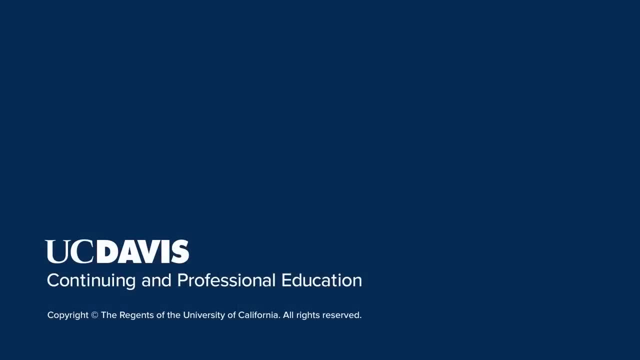 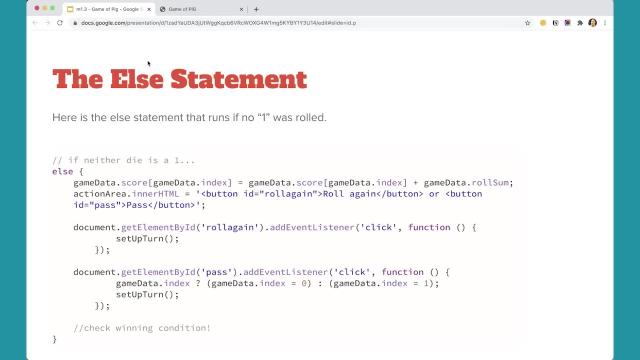 the next thing we need to look at is the final l statement, which will happen if you throw the dice and no ones are rolled, and basically what we need to do is we need to update the score to for whichever player had them. we're going to take the score they had before and add the roll. 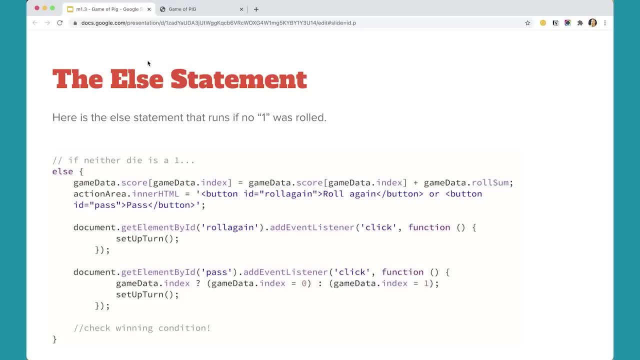 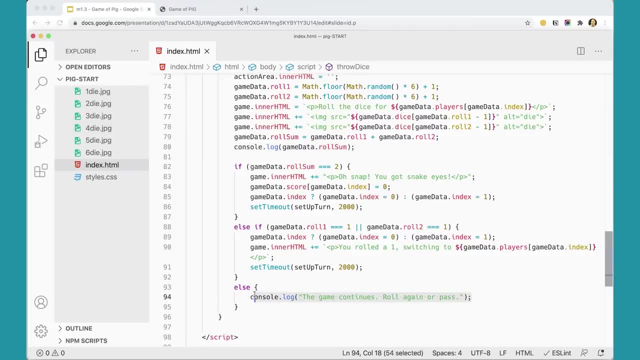 score to the score that they had before and add the roll score to the score that they had before, sum to it in order to update that score. so let's do that first. so we're going to get rid of this and say game data, dot score and the score is going to be for the game data. 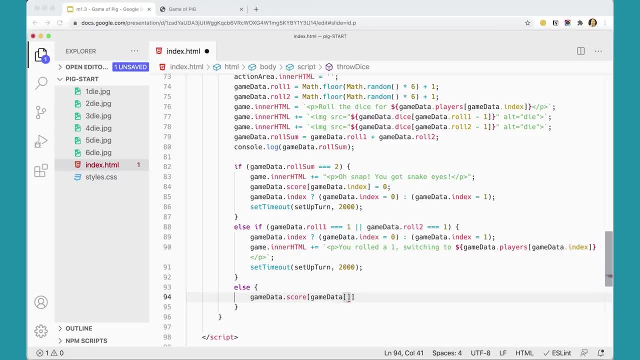 dot player. uh, what is it? sorry? game data. i'm sorry, i'm kind of confused here. game data dot index. that's what i'm doing: square bracket. okay, score for a game data dot index. so that's either that's either game data dot index or game data dot index. so that's either game data dot index. 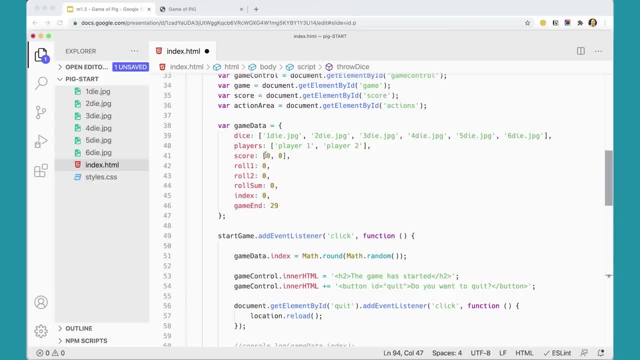 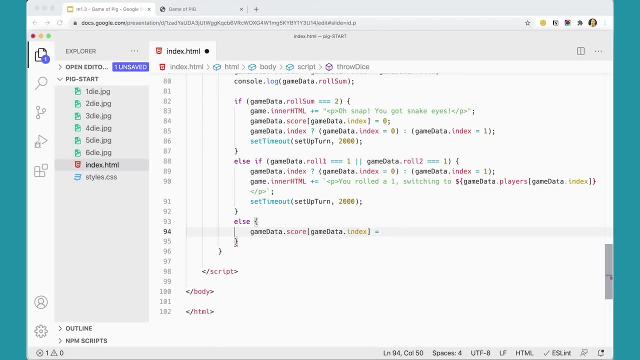 or game data dot index, or game data digit, which is basically my index of four pixels. this score that is going to get me the score. that's the score that i'm going to get me here up here on score. that's going to get me either this one. 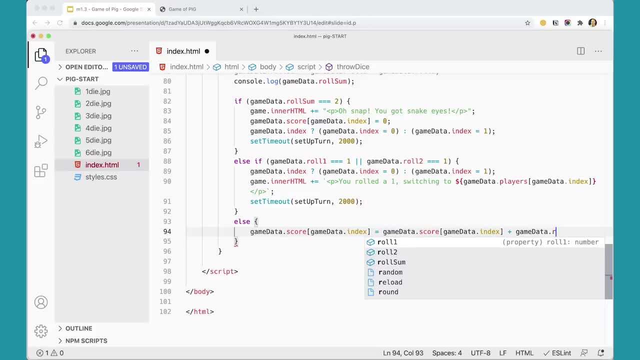 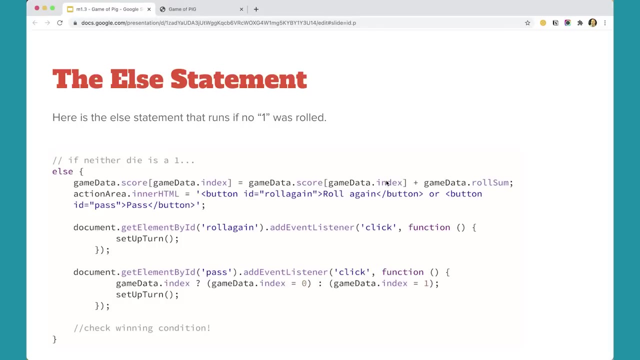 bracket. no gamedatarollsum Like that, I believe. Let me check over here and make sure I did that right. gamedata index plus gamedata roll sum: correct, Okay from there. what we need is to set the action area and create two buttons in there, So that action area is going to get set. 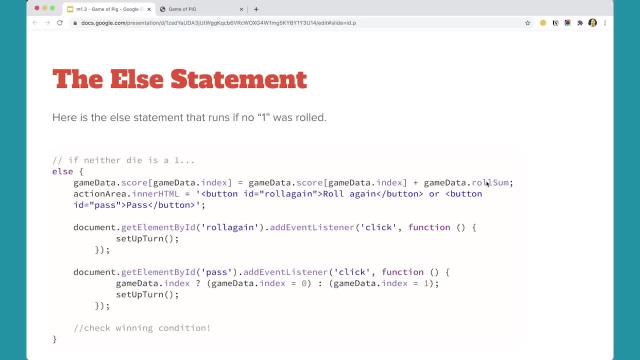 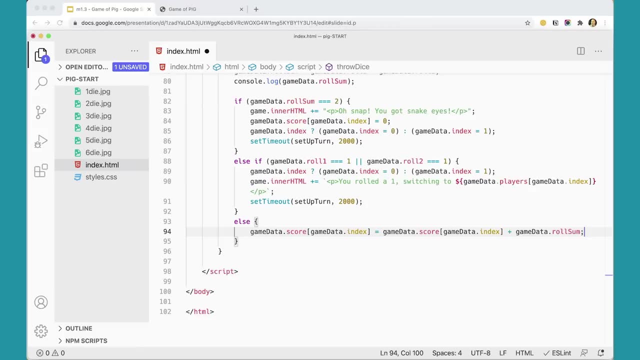 with two buttons, one for rolling again or for passing. So let's go ahead and do that, And that's just simple HTML that we're letting JavaScript generate there. So action areainnerHTML equals open and close quote. there I'm going to have a button: close button. 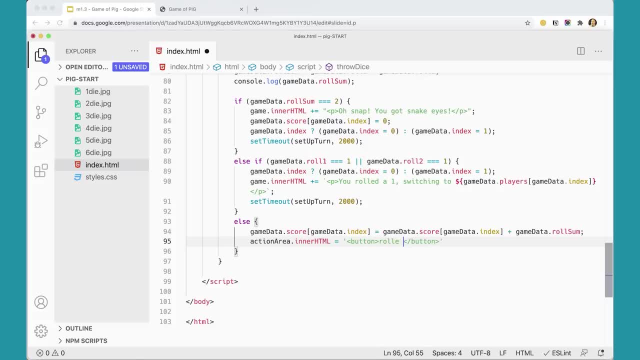 We'll call that roll again And it's going to have an ID equals quote quote, roll again, something like that. So there's that, Or we're going to do another button, Open and close it And in there put pass, And that one's going to have an ID: ID equals quote pass. So you notice. 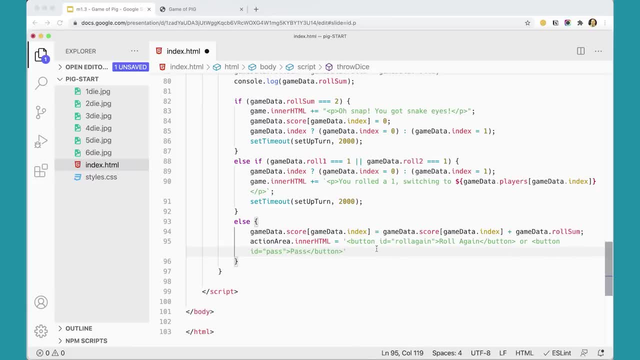 how I do that from the inside out, for even typing this stuff, because that will keep me from making mistakes. That'll help me from making mistakes. I might still make mistakes, but that'll help. Okay, so we're going to set that And then we need to. 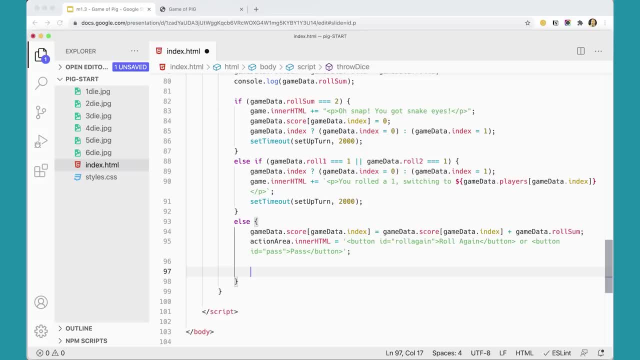 We need two event listeners for each of those things. So I'm going to have an event listener- documentgetElementById- roll again- And that's going to have an addEventListener. I'm listening for a click And when you click the button, we're going to run a function. 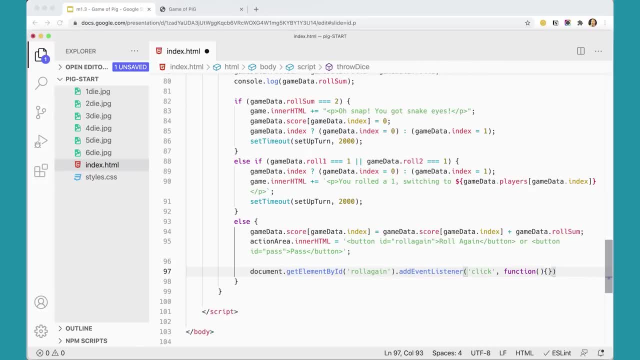 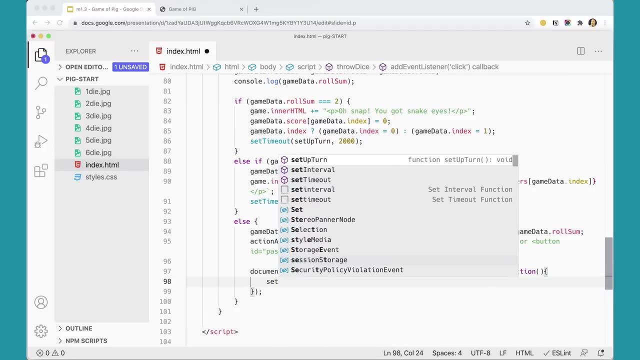 And for now we're just going to put in here: set up turn. We're going to run that function again. Great, So if you roll again, we just set it. When you click that button to roll again, you just set up the turn again and the player hasn't changed or anything. 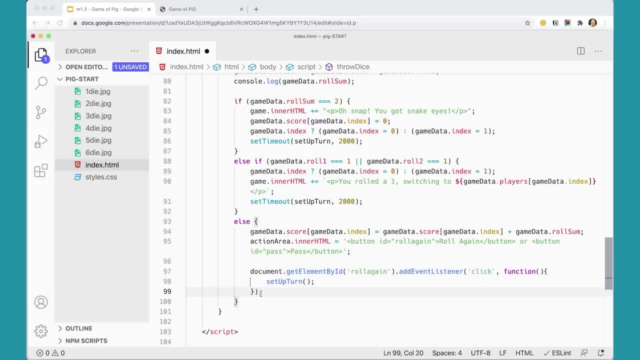 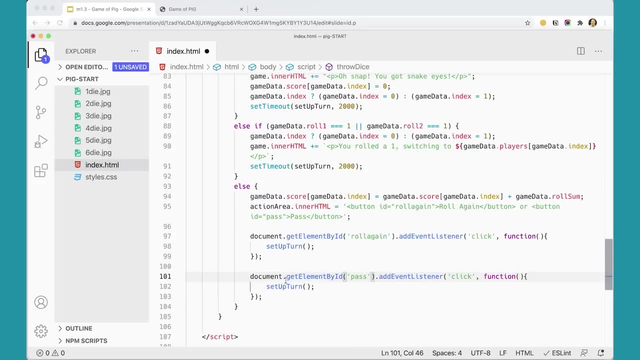 However, we're going to have another one of these And I can just copy this and paste it And change this to pass, And we're going to run, set up, turn again. But before we do that, we're just going to swap the player, So we can just copy that ternary operator and stick it in. 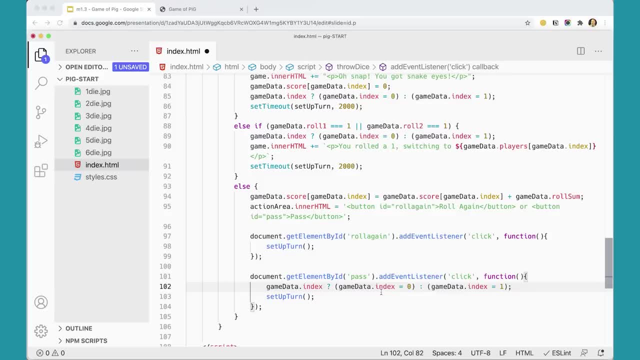 here And that will allow me to swap the player to the other player. Cool. The last thing we're going to need in here is we're going to need something that checks the winning condition. So we'll check the winning condition in here as well, But we'll do that later. 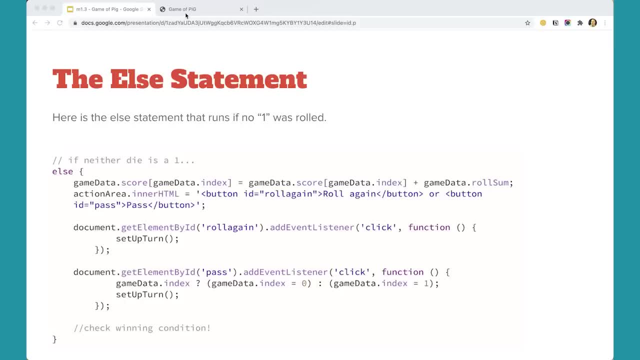 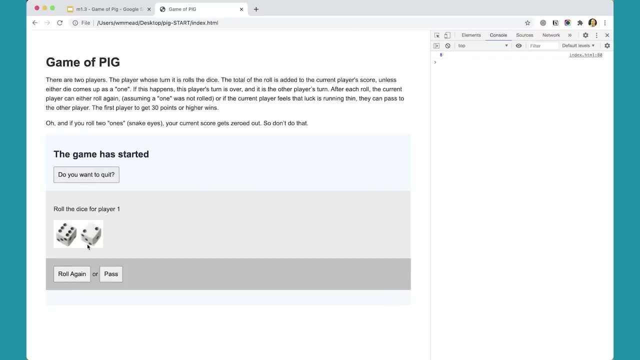 For right now, let's just test this out and see if it works. Come over here, refresh the page, Pick my player. When I roll the dice I get a two and a six. That adds up to eight. I don't have any scoring going on down here yet, but I can choose roll. 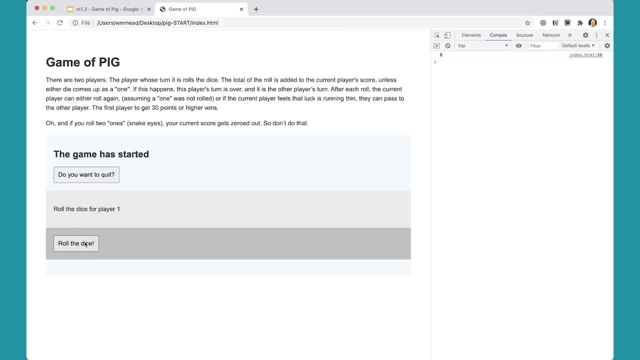 again, And I can just check the winning condition in here as well, But we'll do that later. For right now let's just roll again. And it says roll the dice for player one. And now I've got a one and a. 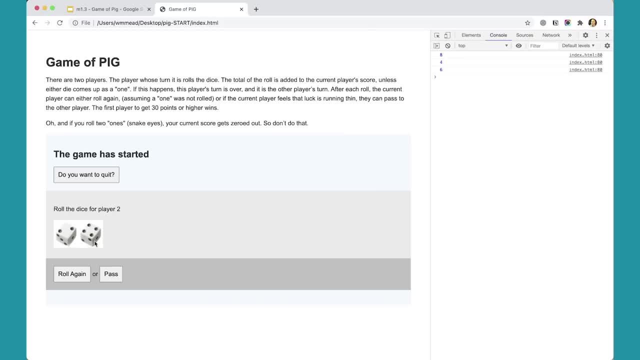 three, You roll the one, switching to player two. Roll the dice. I get a two and a four. I can click roll again And I'm still on player two And I can roll the dice again. Now I've got a five and a. 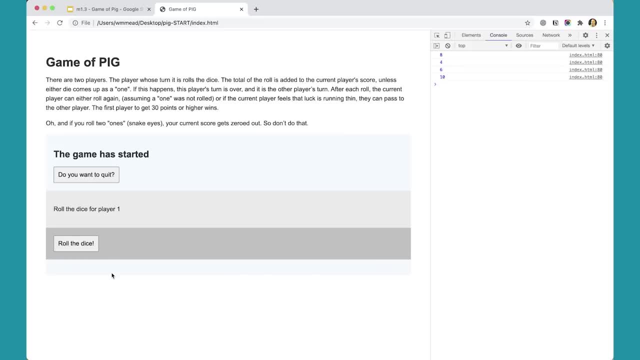 five And I could pass if I wanted to. If I click pass, it sets up the turn but changes it to player one because of that ternary operator And I can roll the dice for player one And I've got a six and I can choose, roll again. So that's all. 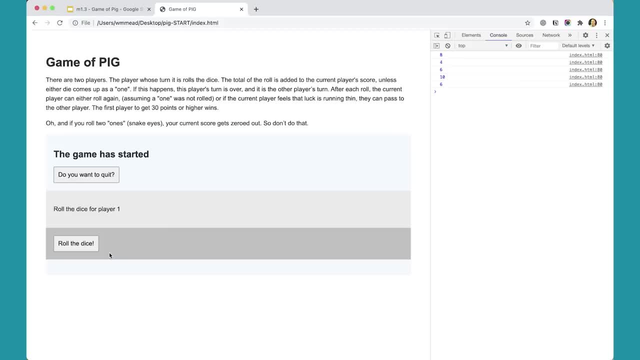 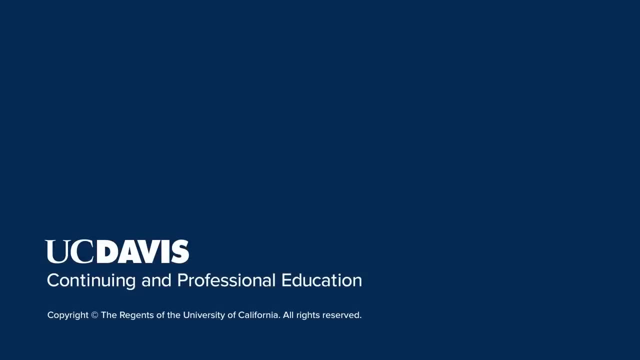 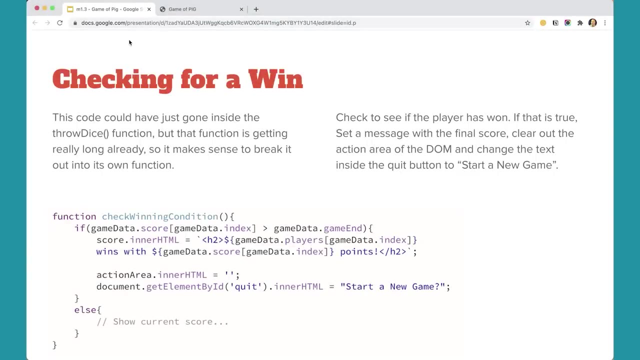 Working great. It's working perfectly fine, just the way it is, Excellent. Let's stop there and we'll pick it up in the next video. The third major function we need is the function that checks for a winning condition: Has the player scored enough points to actually win the game? So let's make a function for that, called check. 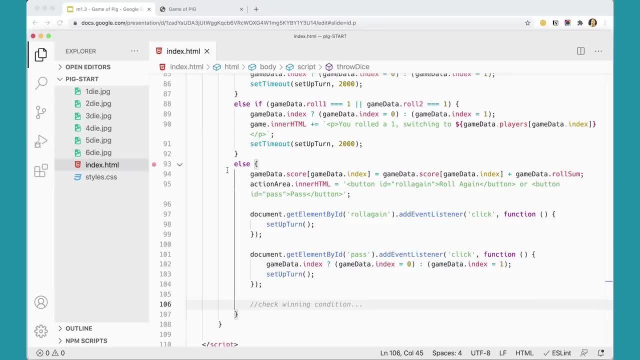 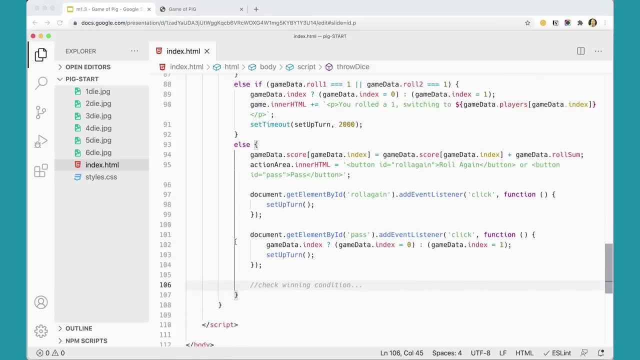 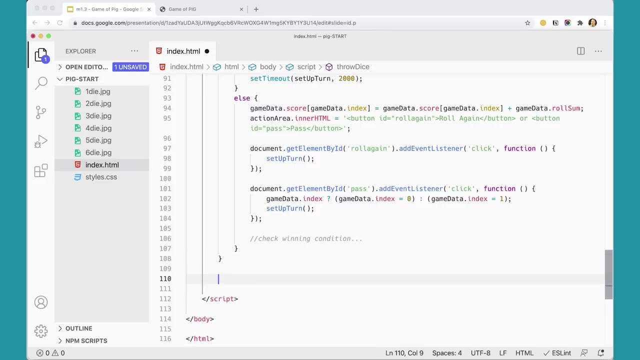 winning condition And add that to our functions down here. So this really long function throw dice goes all the way down to this closing curly brace here. It's kind of a long function And we'll talk about that more in a few minutes. But let's add another function down here, Function check winning condition. 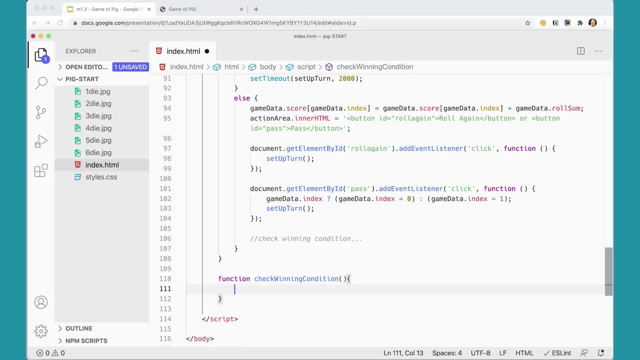 And this is a really long function. So let's add another function down here, Function check winning condition, And this function's going to have an if else statement in it. The if statement's going to handle with what happens if you have actually achieved the winning condition. So if you know, 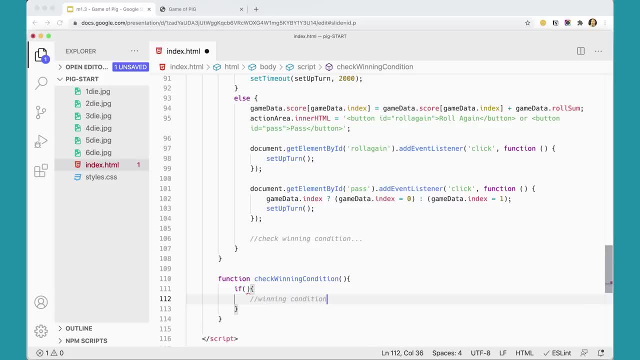 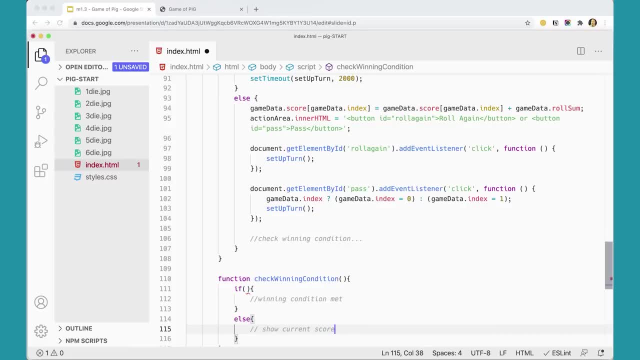 So if we haven't won, we've got to add another one. So if we haven't won, we've got to add another one. Maybe, if we don't win, at least we ought to know well how far along are we, how close are we to winning? 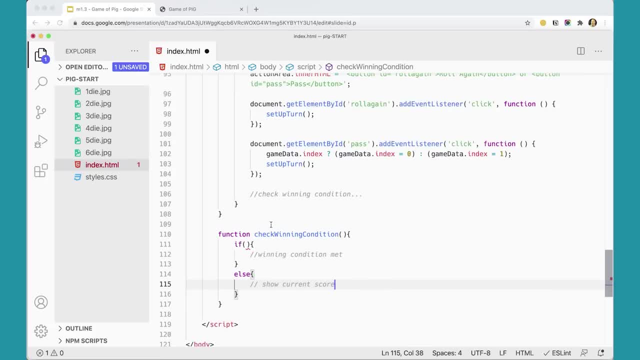 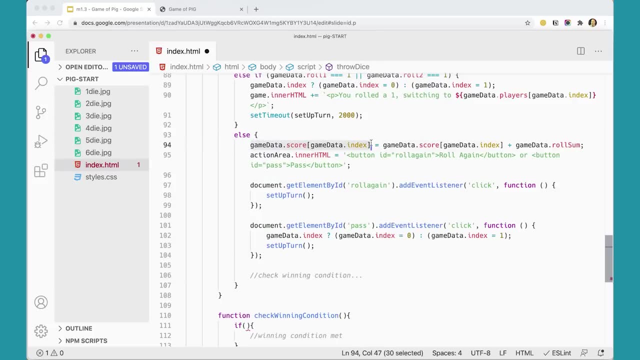 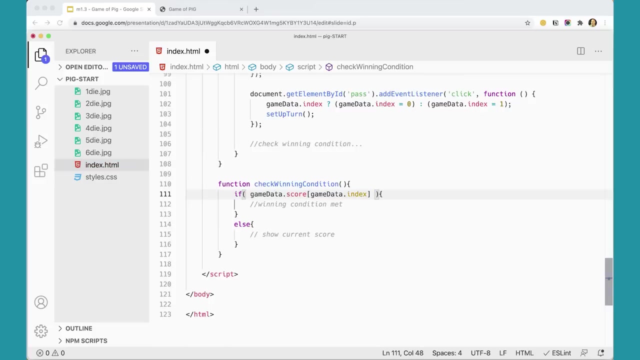 Well, how far along are we? how close are we to winning? So it's going to do those two things. So to check the winning condition, we really just need to get this player's score, Get that player's score And see if it's greater than game data. 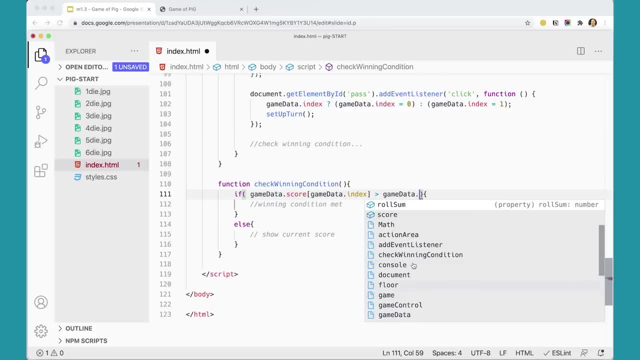 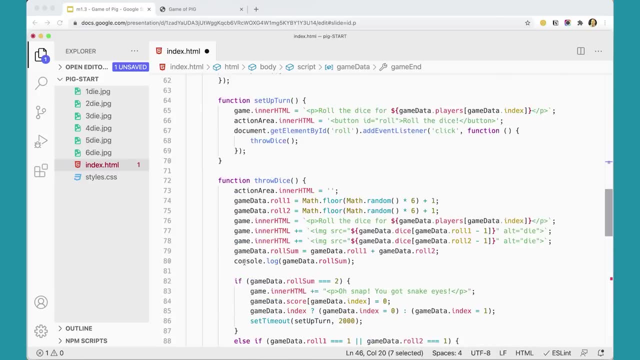 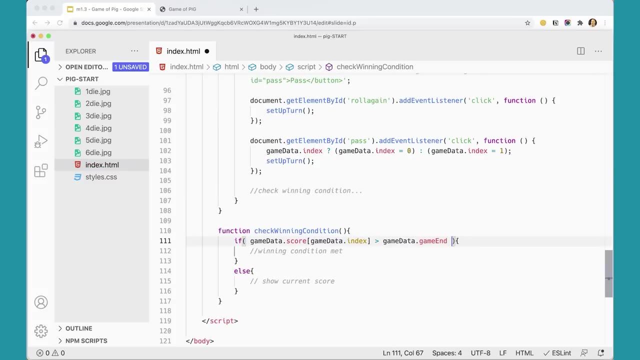 Which one is it? Let's go up here and look GameEnd. Is it greater than GameEnd? Is their score greater than GameEnd? If that's true, then we need to do some things, And what do we need to do in here to make that work? 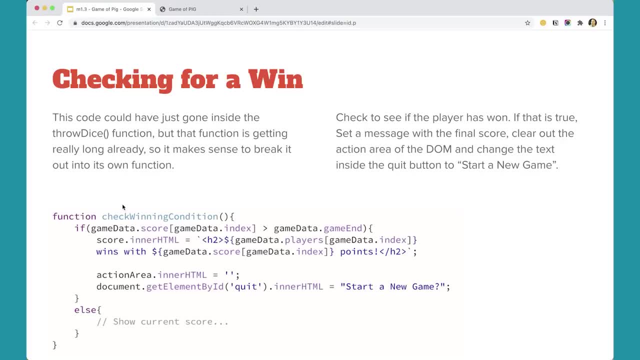 Well, let's go back over here and see We want to set the score area of the page to say this particular player, player 1,- remember, this is going to be player 1 or player 2, wins with what is the score, and then we can say points. 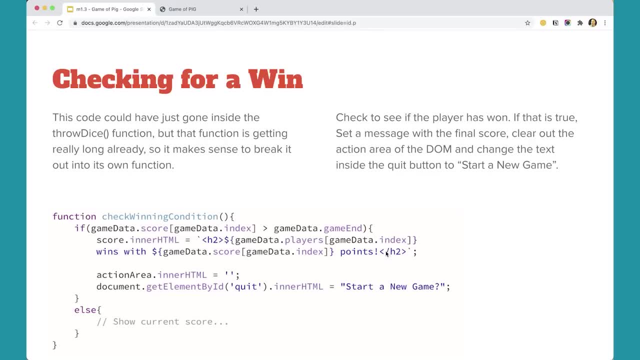 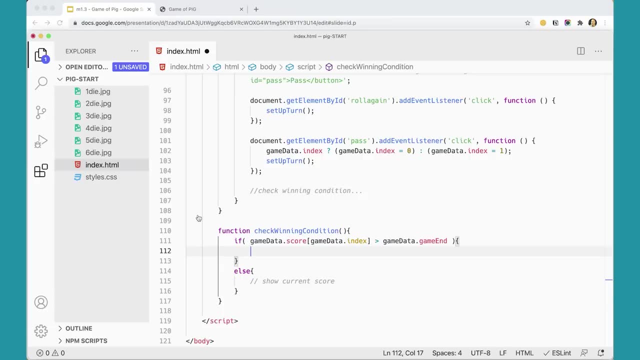 And I'm just putting that inside of an H2.. Notice the tick marks, because we're going to put variables in there, So let's do that. Score: innerHTML equals quote. we use tick marks there. actually tick marks semicolon H2, close the H2.. 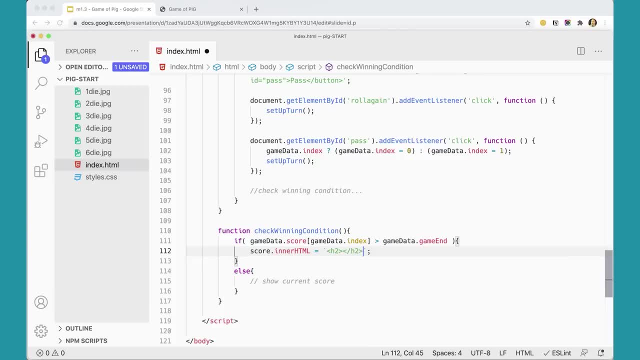 Make sure you type it this way. It will be much better for you if you do. Player X wins with X points, Something like that. But player X is going to be a variable, So we're going to do dollar sign curly braces. 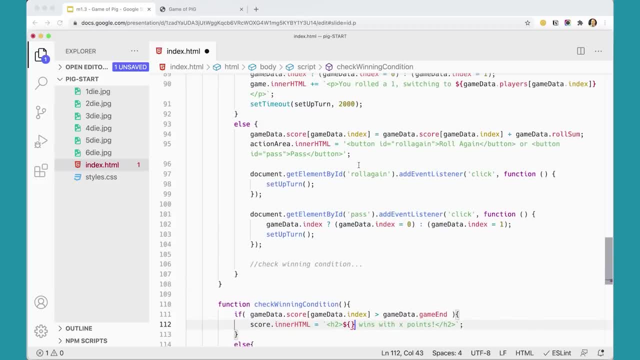 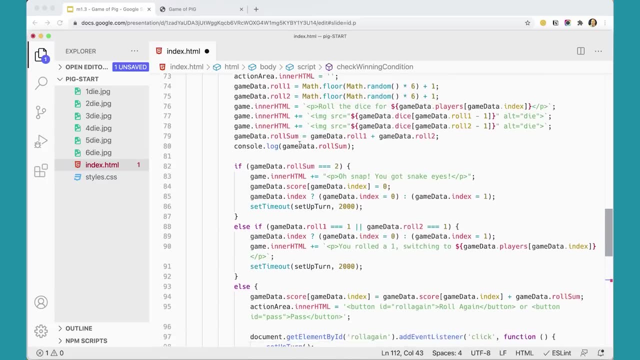 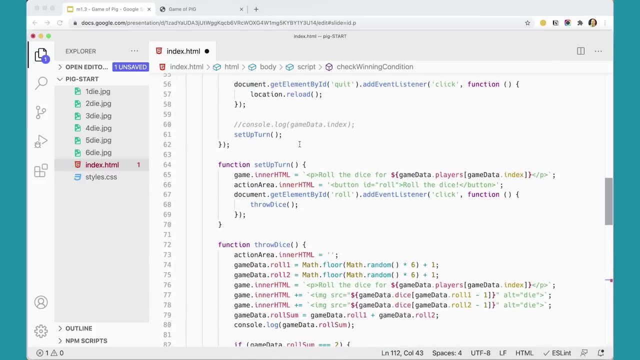 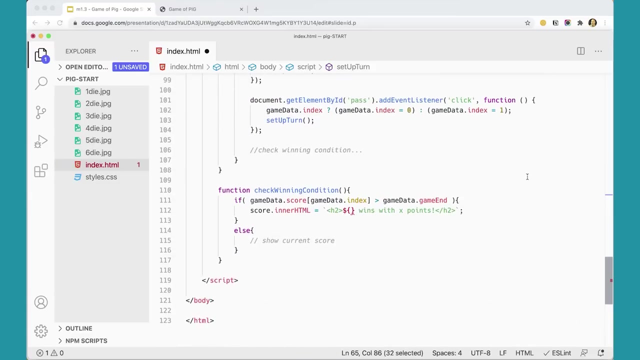 and in there we're going to say: where's my player thing? I'm going to switch players. It's up here: Game data players, This one here. Other than typing, it's nice to copy and paste, So stick that in there. 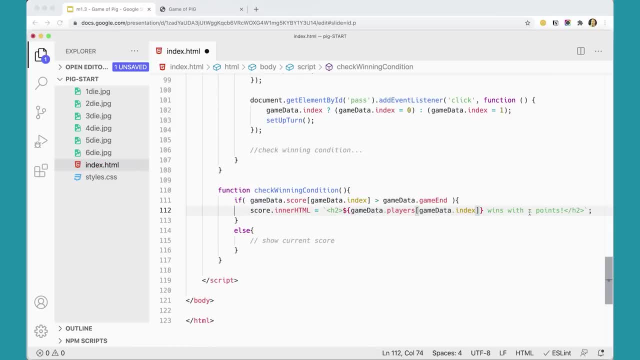 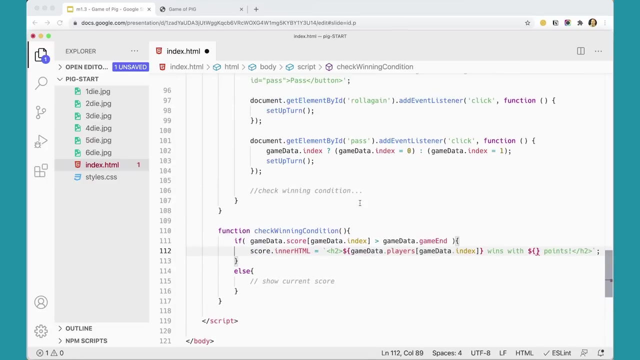 So that's going to be either player 1 or player 2.. Wins with X points. So that's going to be another variable there. Curly braces, Sorry, dollar sign, curly braces. And in there goes this game data score. 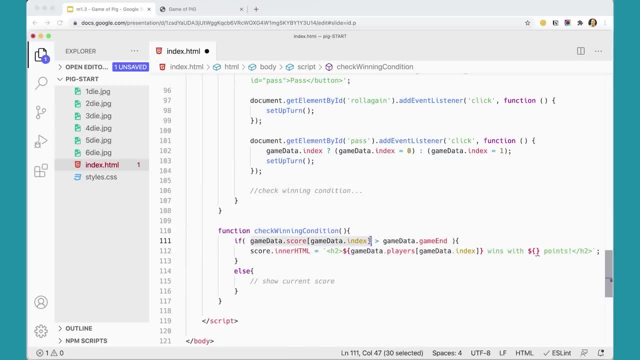 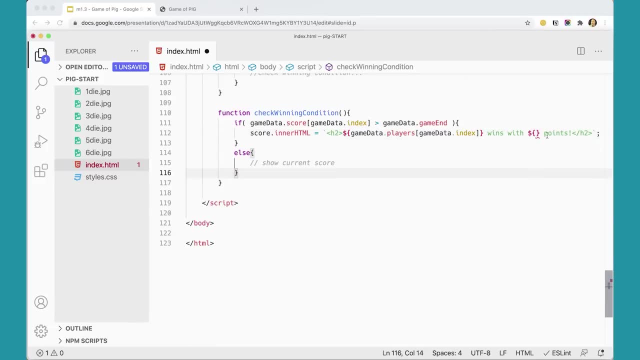 Index This thing here, Because that's the score that we got, So I'm just going to stick that in there. Whoops, I'm going to click on that, So that goes inside the H2.. That's great. What else do we need to do? 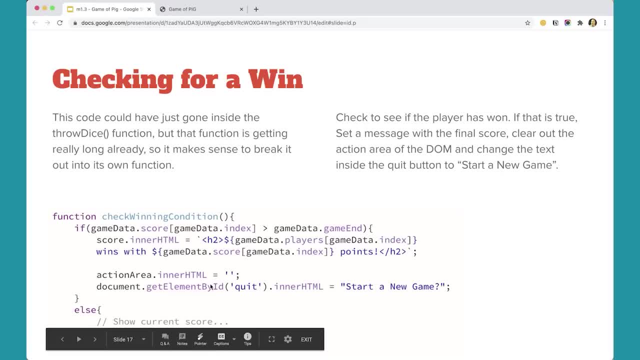 I'm going to clear out the action area And then I'm going to make a. I'm going to get element by ID: quit That button that's up at the top of the page. I'm going to set its inner HTML to starting a game. 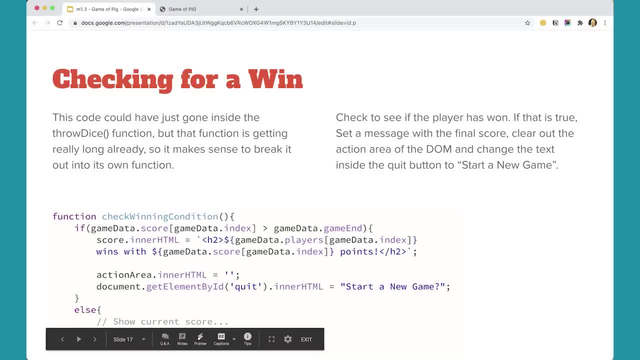 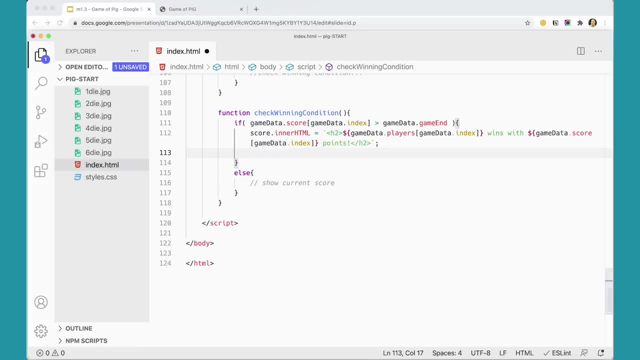 So let's just do that: Action area equals quote, quote. We're just clearing it out, That's all we're doing there. And then we're going to say document dot, get element by ID, quit, So that button. there I'm going to say it's inner HTML. 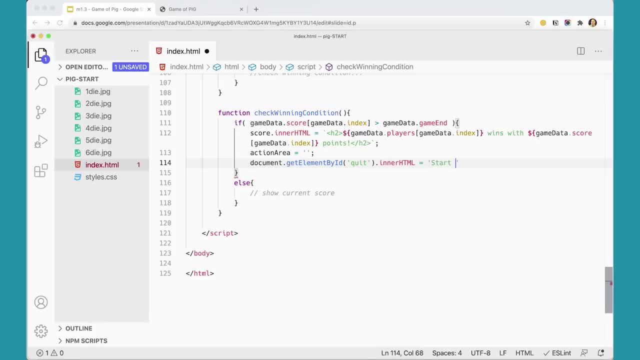 It's going to be start a new game, Something like that, So that once we've won, we can start a new game. Cool, So that's the if statement. That will check to see if the game has won. we will start a new game. 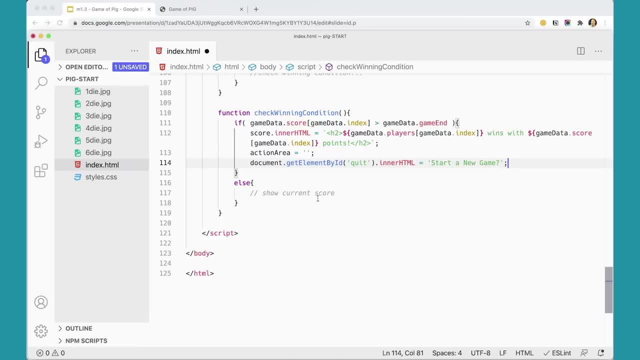 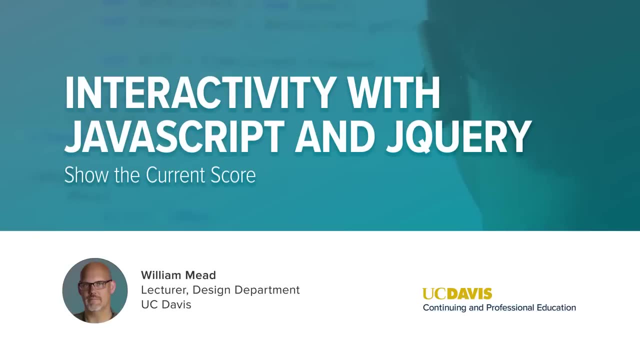 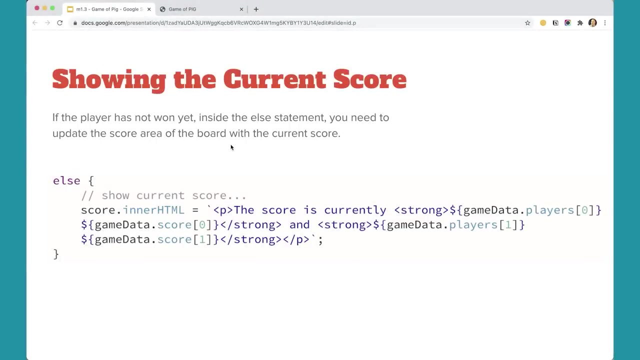 In the next video we will fill out the show current score section of this function. Okay, So now we need to show the current score and make sure that that gets filled out properly. if we haven't won the game, So let's go over and add this. 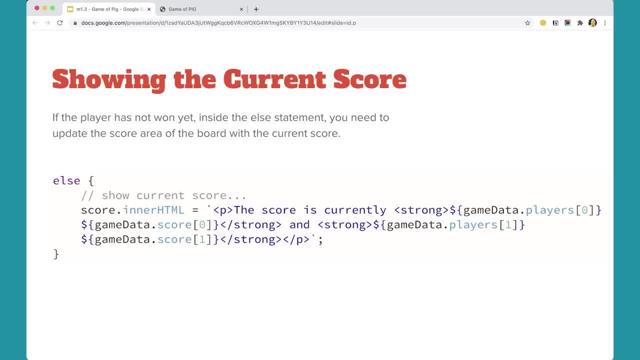 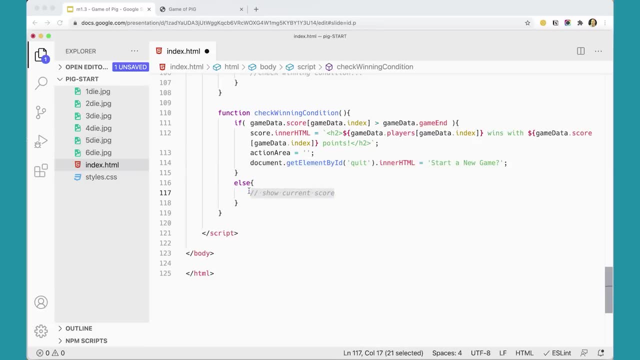 So basically we're going to set the score areas inner HTML to a paragraph that shows the scores of both players. So we can say score dot, inner HTML equals, and I'm going to just put in here some tick marks and a paragraph like so: 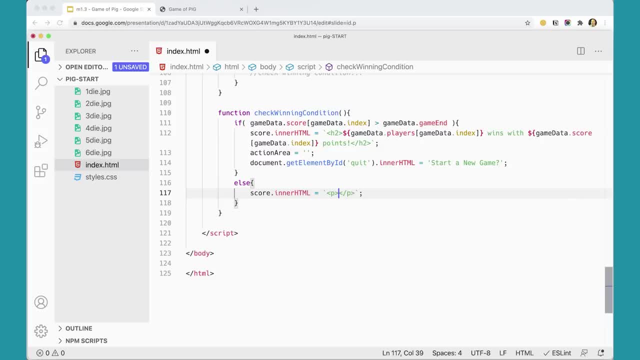 And then in here I'm going to say something like: the score for player one is X and the score for player two is Y, something like that. Now, player one is going to be replaced with a variable Curly braces, whoops, dollar sign. 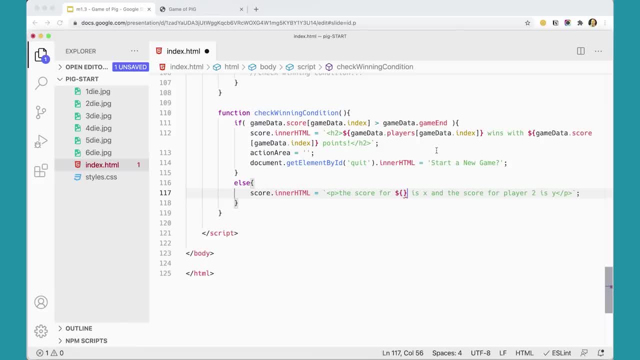 keep down that dollar sign, curly braces. And again, player one is this thing here, player's index. I just need players game data. players: square bracket. zero is going to be something, And what score is that going to be? This is going to be a variable here. 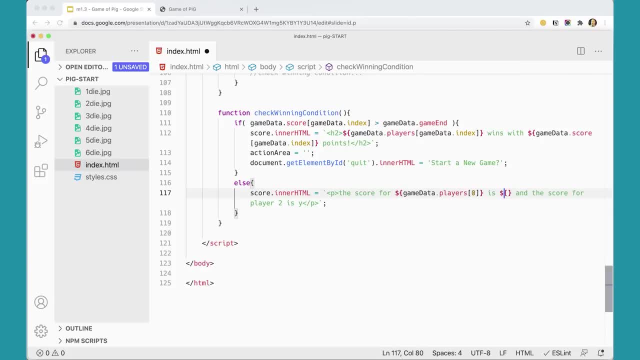 Curly braces. And again, I forgot the dollar sign. And in there we're going to say game data, dot, score, square bracket zero. So that's the first player's score. And then we're going to do the same thing down here. 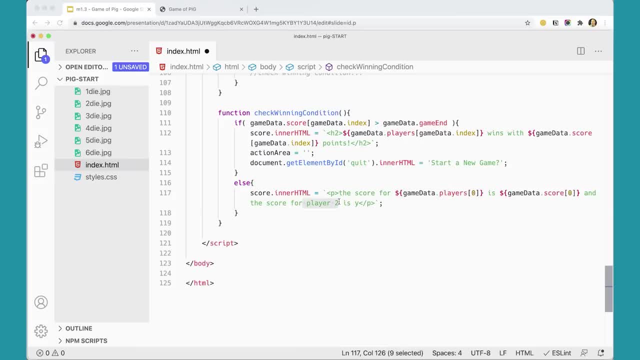 for player two, except that's going to be a one. And this is going to be the same thing down here, except that's going to be a one. And you could even make it stand out a little bit more by putting a strong tag around each of these things. 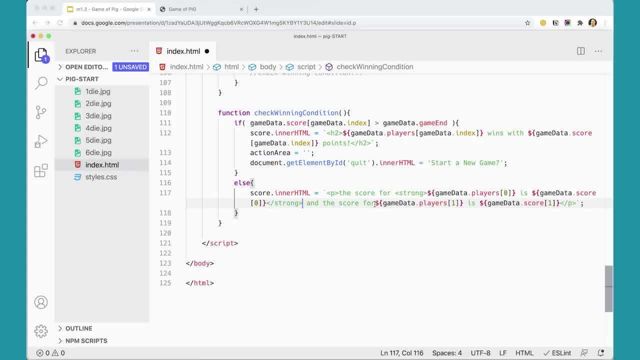 And you could do much better than this for coming up with sort of a nicer interface for this. but, But this will take care of us for the moment. There we go, So we're going to put that into the score and then we're ready to continue. 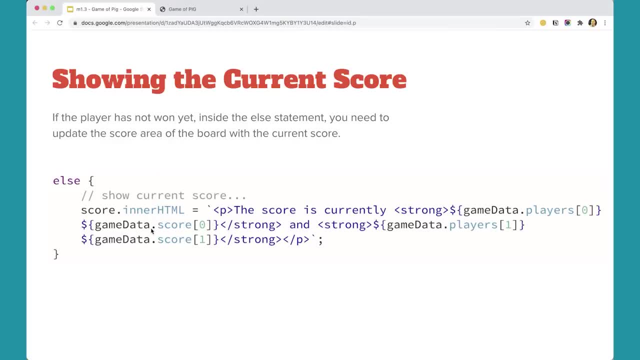 I believe that's all we need. Let's just see over here: Yep, Player, zero player. one looks good. That all looks good, All right, great. So what do we need to do to get this to work? We need to run this function. 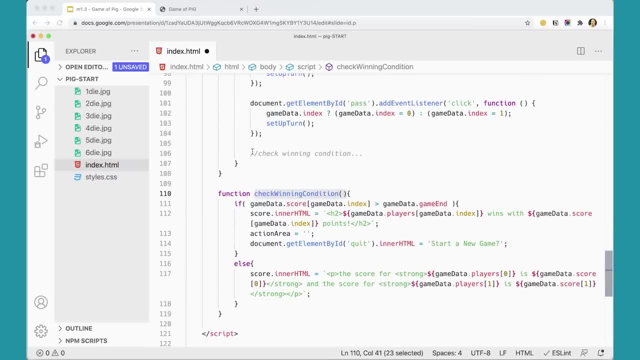 Here check winning condition. It's not the only place we need to run it, but let's start with that, Let's put it there, Let's test this. Make sure you save the file, and I'm going to come over here and refresh my page. 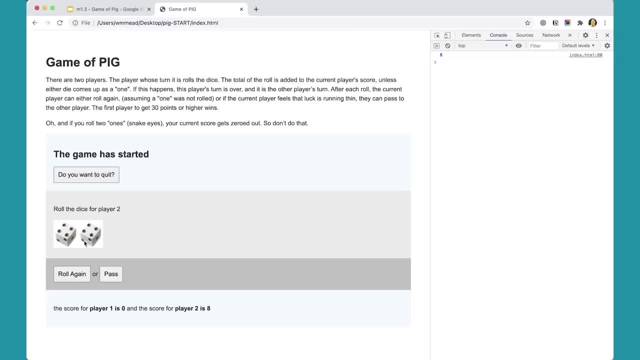 and start my game, Roll the dice for player one. So now I've got eight and I'm going to run it And I've got No. player two is running here And you can see that the score got added up. 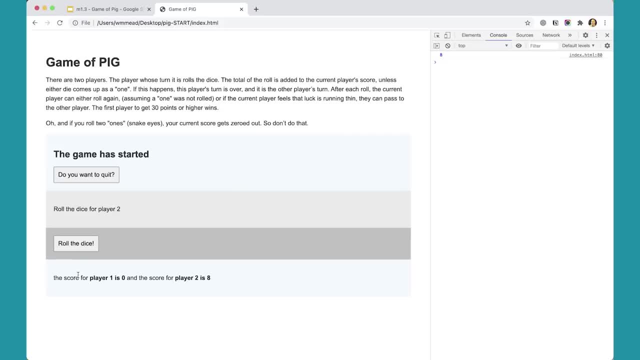 Player two has eight points. I can click roll again And it takes me to set up the turn And I can roll the dice for player two again And I've got 15.. Okay, so player two has 15.. I can roll again. 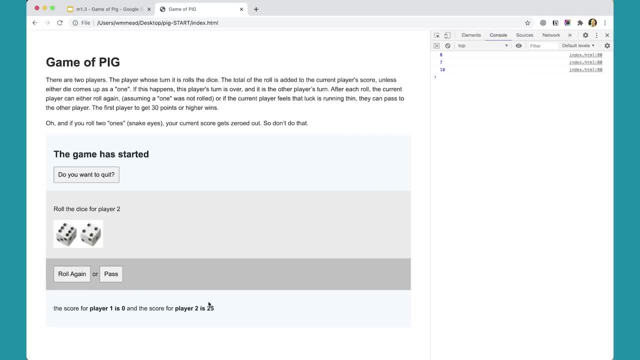 Roll the dice again. It takes me to set up turn. Now I've got 25.. And if I get five or more we should have the end of the game. That should trigger it. So let's see what happens. Roll the dice. 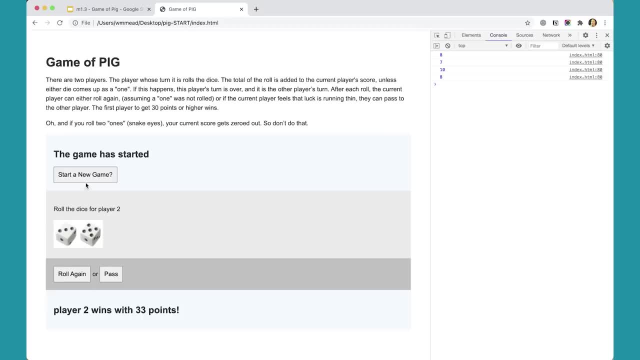 And player two wins with 33 points. And now up here I have start a new game. It still says roll again or pass, so that's something that needs to be dealt with, But we can start a new game up here. What happens if I click roll again? 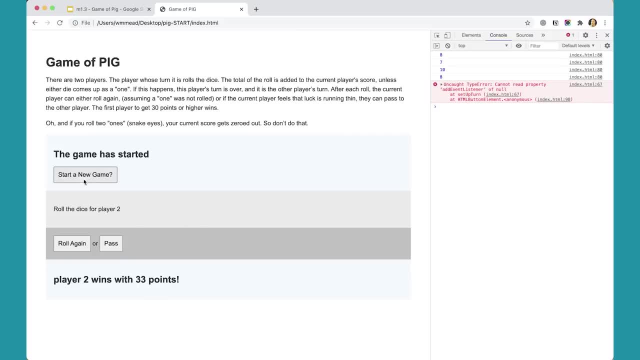 Now I've got an error up here, So that's something that we need to deal with here. Roll the dice. What if I choose pass? If I choose pass, it says roll the dice for player one. Roll the dice. And now I've got a one. 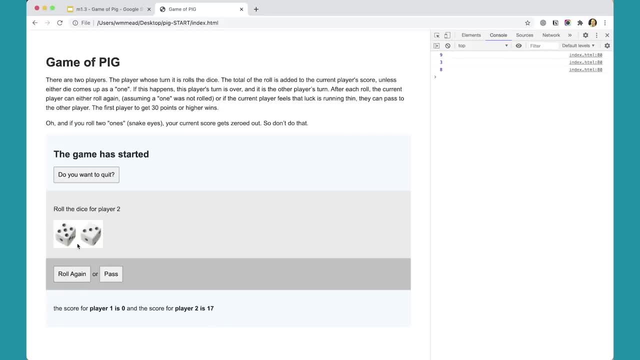 so it's going to wait two seconds and set up for player two And I can roll the dice for player two. So there are a couple things that we want to fix here And one of them that's less obvious because we haven't done it yet. 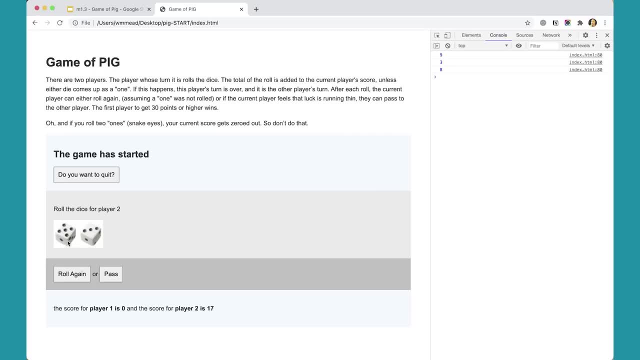 But if you roll two ones, you also need to- um, you also need to- uh, to fix that there as well. So that, because that's going to change the score, So we want to show the score if you roll two ones. 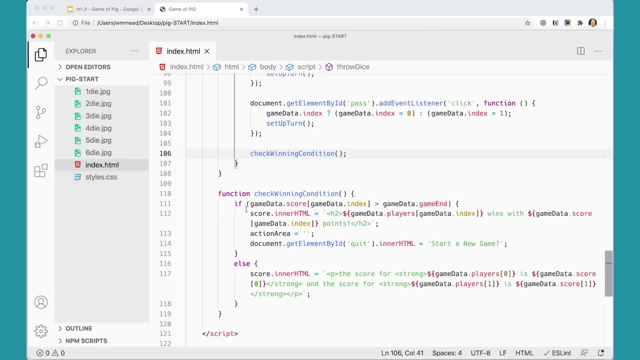 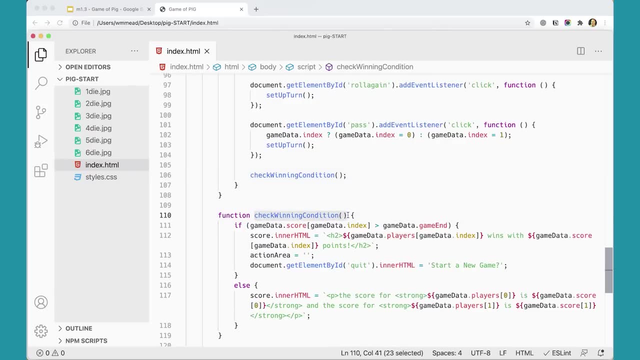 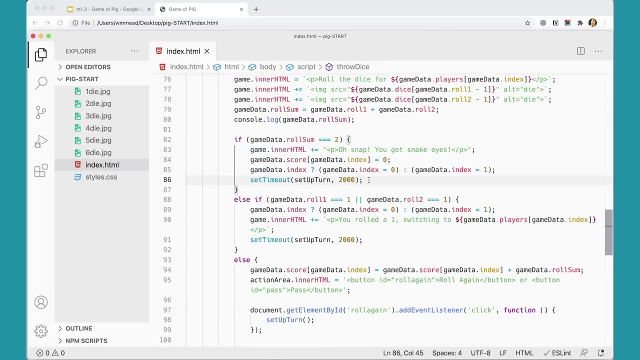 So let's go back to our code over here And I want to run check winning condition up here. if you roll two ones, I'm going to run it here as well, Because because that's not going to have a win, You're not going to get a win if you roll two ones. 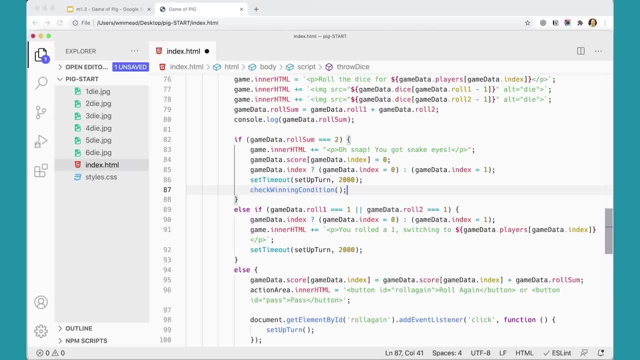 But the score is going to change. So, um, if you roll uh two ones, then that player's score gets zeroed out, And you want to be able to see that, So we'll put check winning condition there as well. 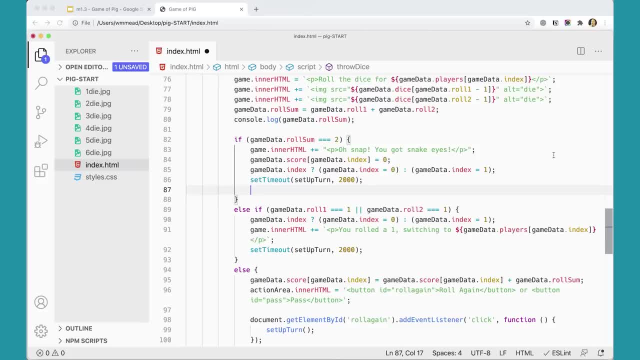 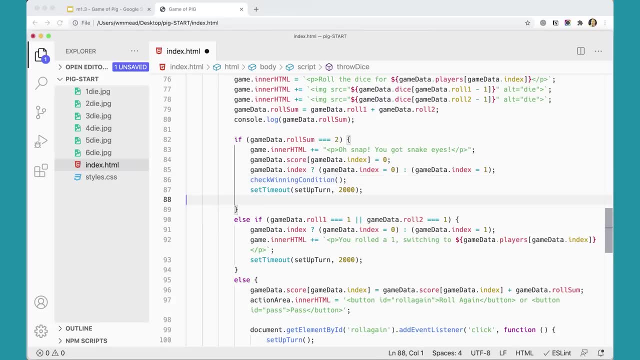 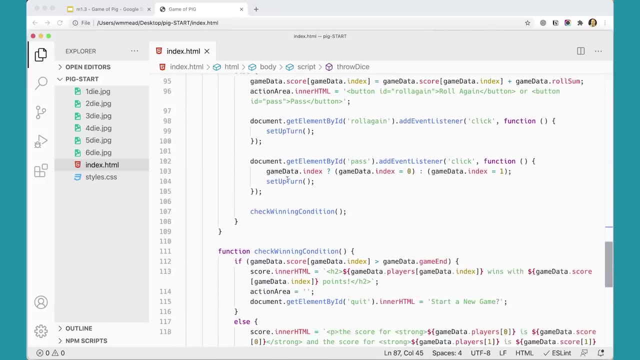 Actually, we'll put it before the set timeout Doesn't actually matter. The set timeout will wait two seconds anyway, But, um, I'm going to put it before that. There we go. So that helps. The other thing we need to do down here is that. 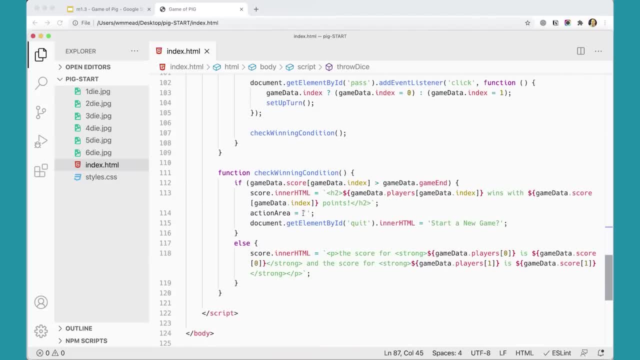 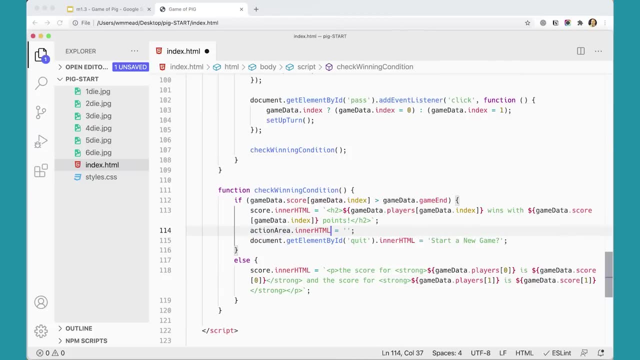 um, if you've won the game, I'm setting the action area. Oh, actually, this is what I'm missing. Dot innerHTML. That's what I was missing from before. Action area innerHTML. set that to blank, so that that'll get rid of those buttons that I have there by accident. 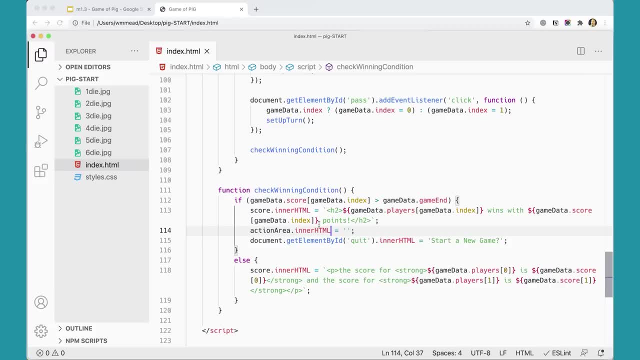 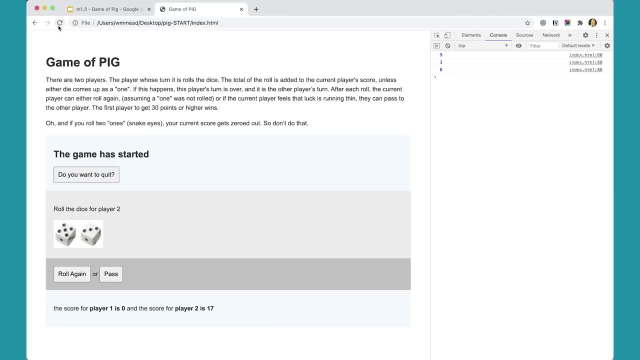 Now there's one more thing that we can do to make this work a little bit better, but let's just test this again, just to make sure it's all working right. Roll the dice, Roll again, Roll again, And that's working. 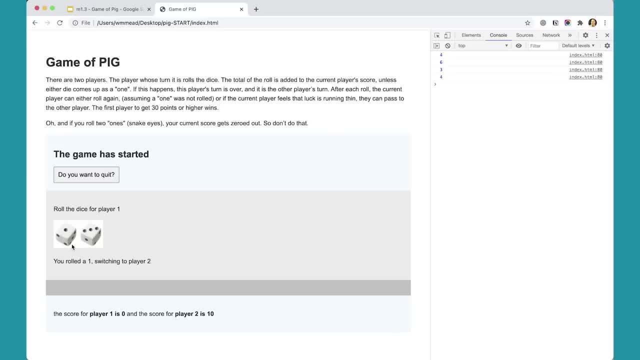 And then, uh okay, we got switched to the other player. Oops, got switched back. Poor player one is still at zero. We're rolling Well lots of ones here, just by pure random luck. Kind of nice if we rolled a double one. 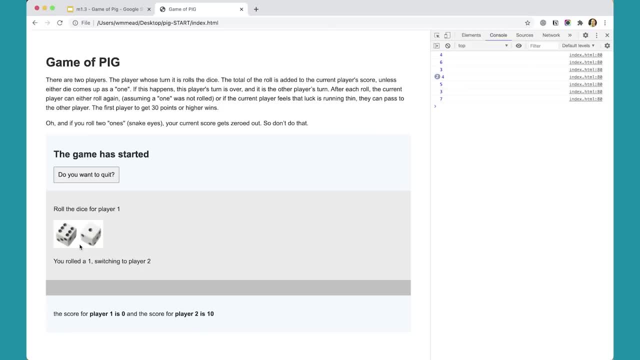 All right, finally, player one is on the board. Oh sorry player one. And if we roll again, Oh sorry player one. Oh, sorry player one. Oh, oh, oh, oh, oh, oh. 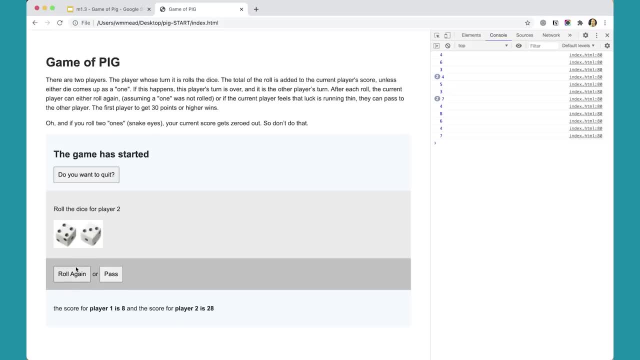 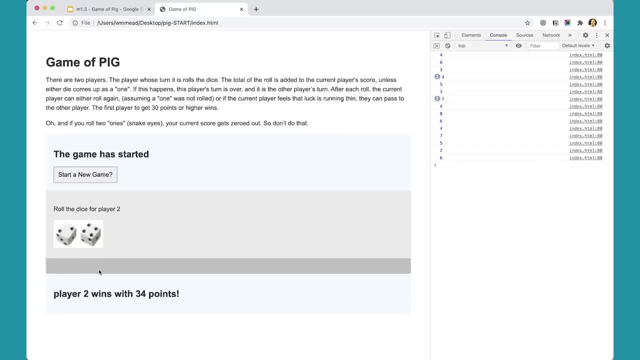 Player one's having a bad game and player two wins, And then we don't have the buttons there, because we cleared that out properly. The only thing you can do is start a new game. So that's all working perfectly fine. so that's great. 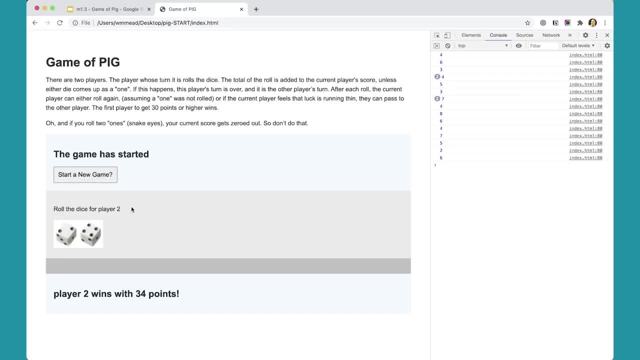 Um, we will stop this video here, but in the last video we'll talk a little bit about a little bit about some things that we could do to kind of clean this up a little bit more, which is just kind of final cleanup stuff. 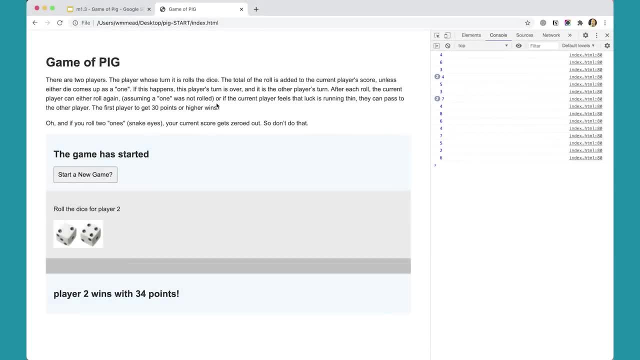 Okay, the game is working, and that's great, And everything is working the way it should, so that's excellent, But there's one thing that I would like you to notice, which is that when you roll the dice for the player, 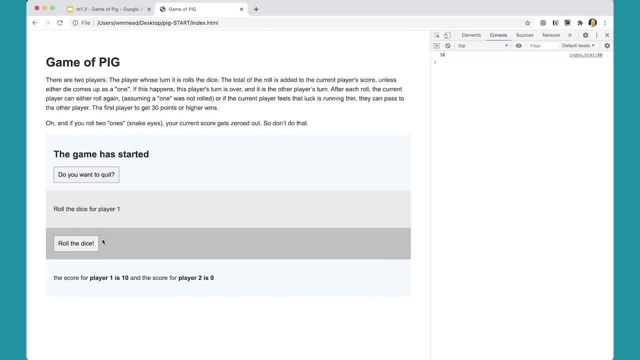 when you roll again. it's going to set up turn which says roll the dice for player one. But it'd be kind of nice if- whoops, I got snake eyes there. It'd be kind of nice if, when I roll the dice again, 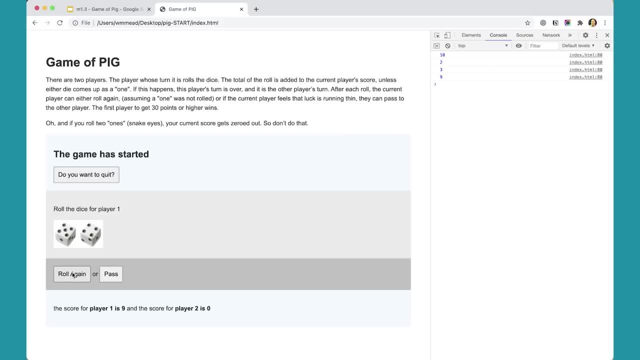 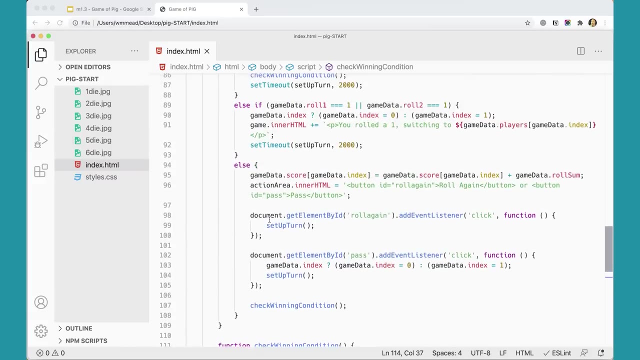 if I click roll again, it just rolls them again. I don't really need to go back to the setup turn at this point. I could just roll the dice. I could roll the dice again. So what can we do about that? What if, down here in the, in here, when we go to roll again? 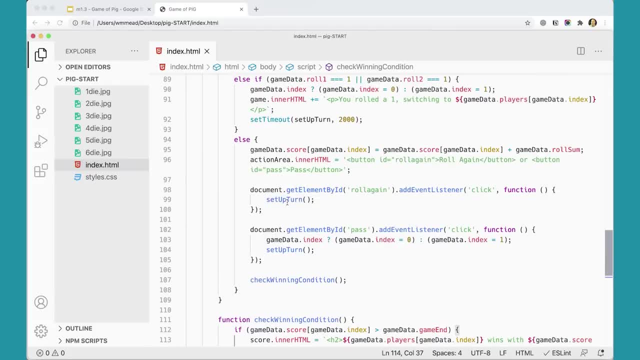 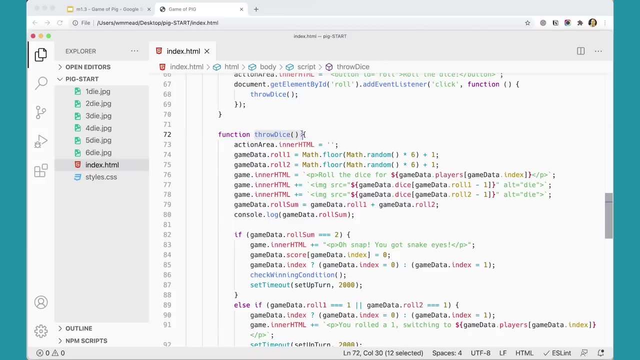 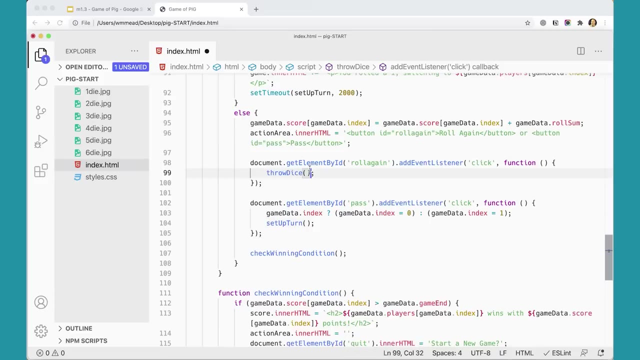 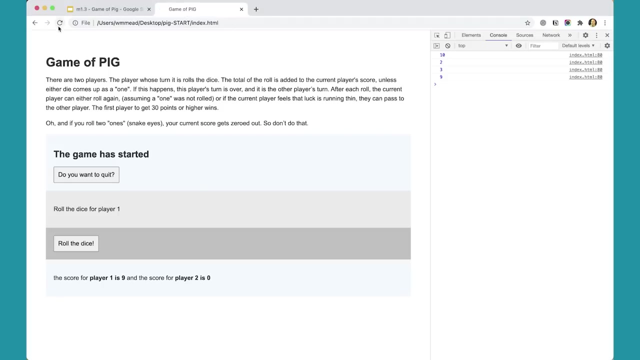 instead of doing setup turn. we just run this function: Throw the dice instead of setup turn here. I think that will work, so let's go back and test that. So now, when I start the game and I roll the dice for player two, 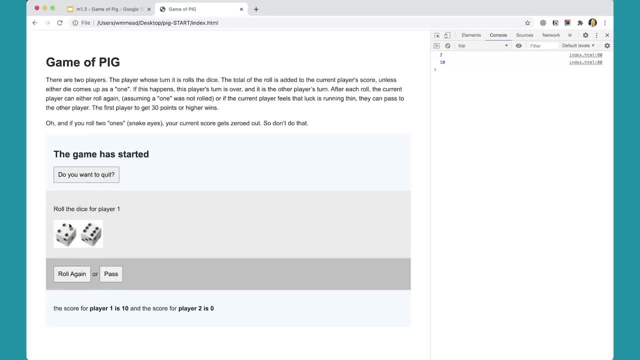 whoops, I got snake eyes again. There we go. Now. when I click roll again, it just rolls again and you can see that the score is getting added nicely. It's a bit smoother, So that works great, Okay, So there's that. that's. that's working pretty well and that's great. 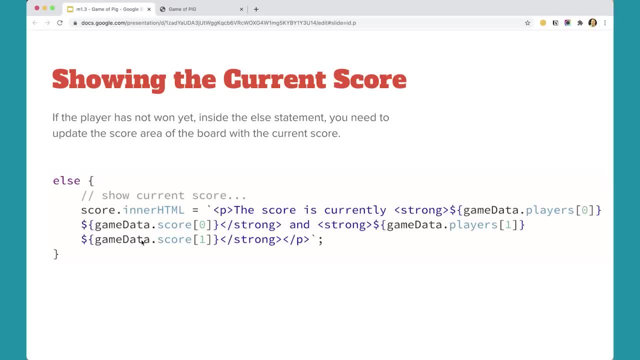 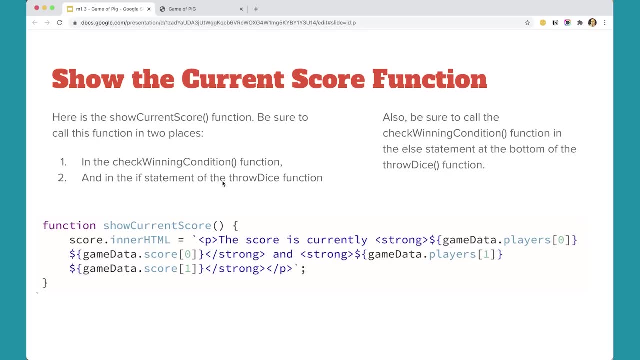 A couple other things to clean up. This thing here is really long and you could turn it into a separate little helper function. I don't know if it's really necessary, but you could make a function called showCurrentScore and make sure you put it in. 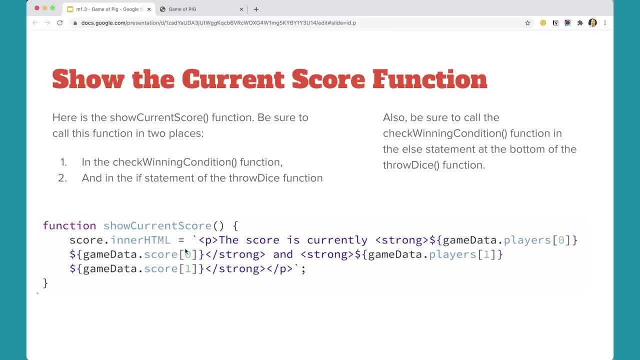 the winning condition and you could move it also into the if statement for the throw dice. Um, we could, we could put it in a couple of different places here. So, let's, let's go ahead and do this, just to see, you know, just kind of. 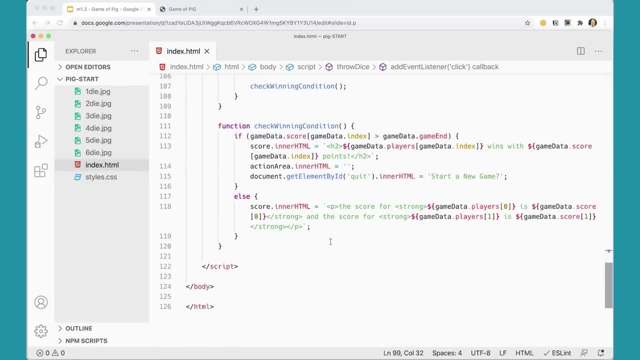 like a little helper function here. So I'm going to say, say, function showCurrentScore and it's really just going to be this stuff, just cause it's kind of long, And then really all we need to do is run this function here. 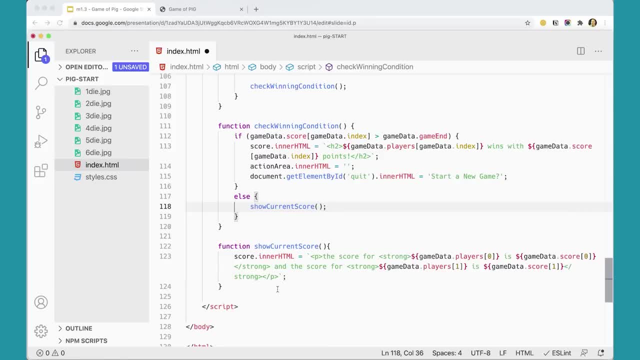 ShowCurrentScore, So that makes that function a little bit shorter. We've just split this thing out Also now. also now we don't need to run check winning condition up when you run snake eyes cause. you're not going to win there, but we need to run showCurrentScore. 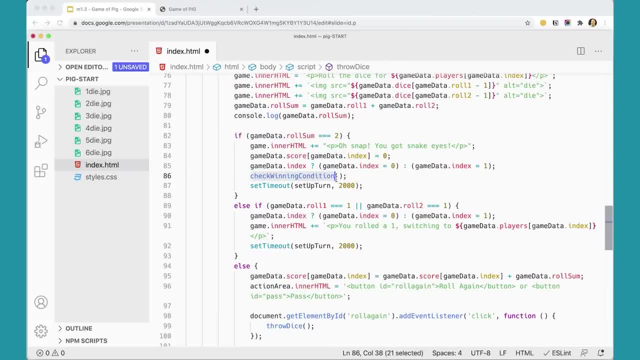 So up here, instead of check winning condition, we can change this to showCurrentScore, And that will actually. that actually makes a little bit more sense, Cause that's what we're doing here. We're showing the current score. Nobody's going to win when they roll two ones. that's going to zero out their score. 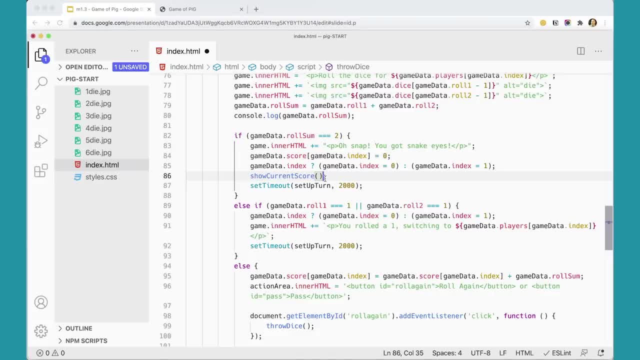 And we want to show the current score. but we don't really need to check the winning condition. We don't need to do the top part of this if statement here. We just need to do this bottom part, which is showing the current score. 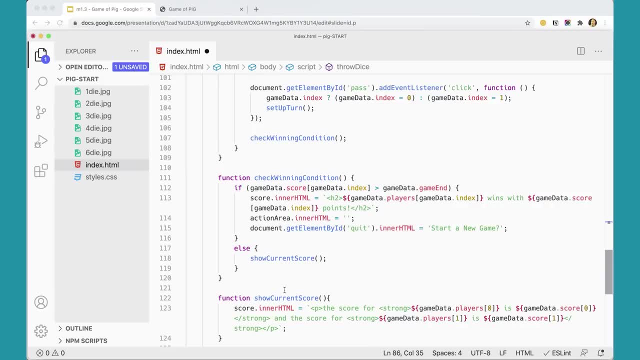 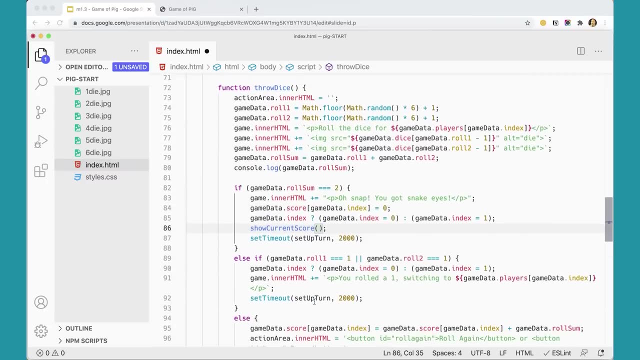 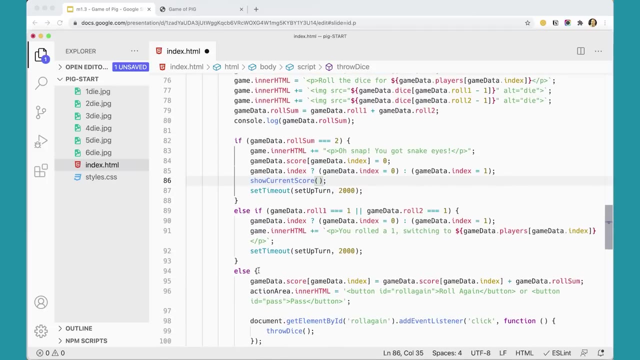 So that's a little bit cleaner and a little bit nicer like that, I think. the next thing I wanted to talk about is this throw dice function is really long. Now you could potentially break out these if statements into separate little helper functions to get it to be a little bit shorter, since none of the 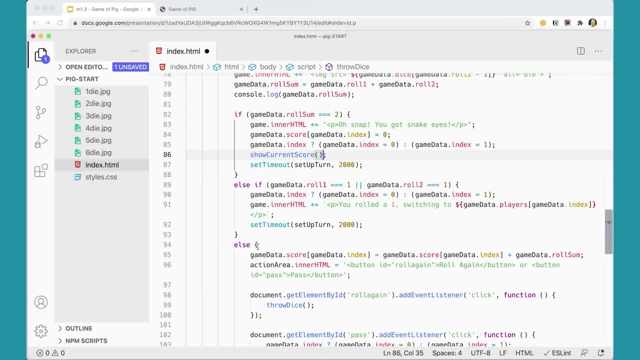 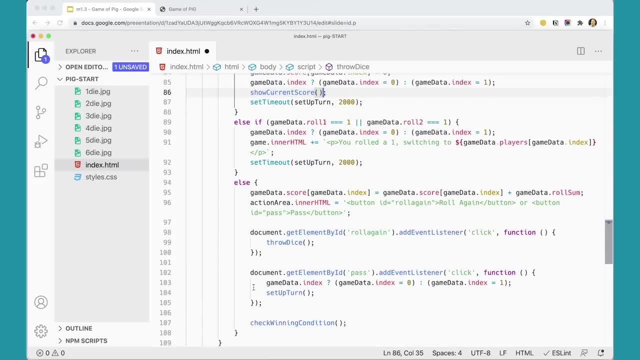 this stuff is going to be used more than once. There's not really a huge reason to do so, So I'm going to leave it the way it is. but you could think about what you would do to create little helper functions like this one down here and 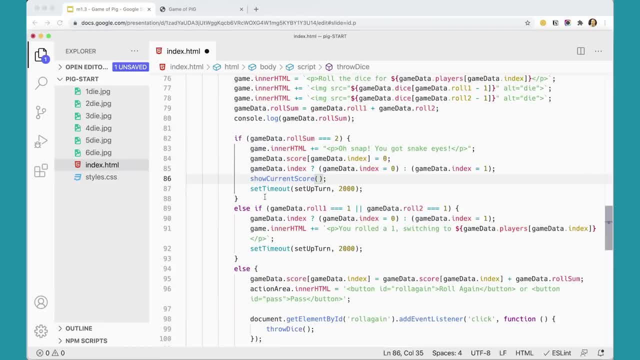 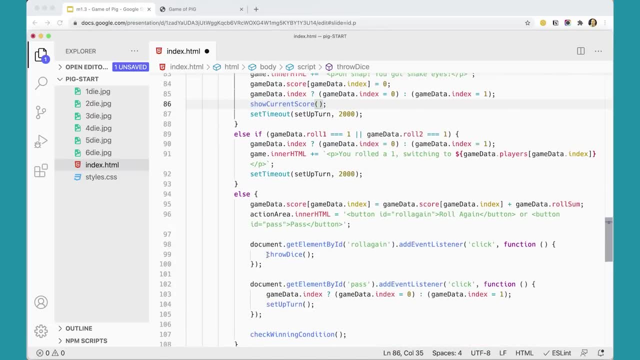 run them in these if else statements, basically pull the guts out and put them in their own separate functions. And you might want to try it, just to kind of get used to working with that kind of idea, and it would help make that throw uh, throw dice function. 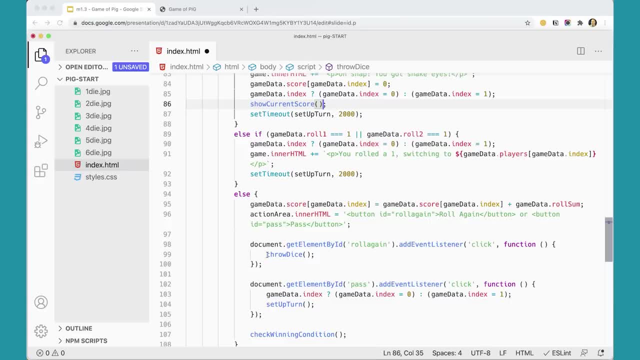 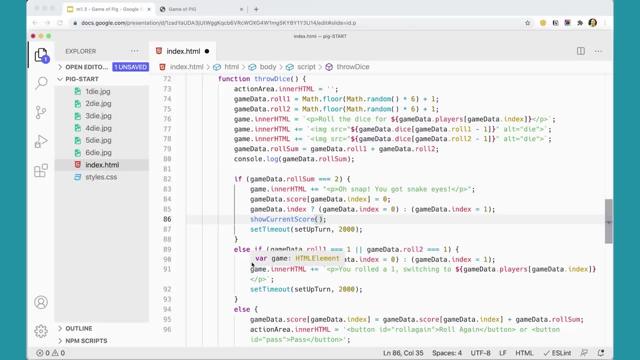 a little bit shorter, which would be kind of nice as well. Um, you could also make a separate function that just contains the whole selection statement, if, if, else, if, and in the else statement, and make that into a separate function that runs here. 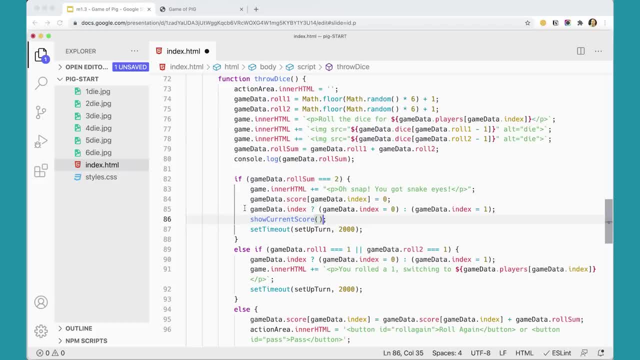 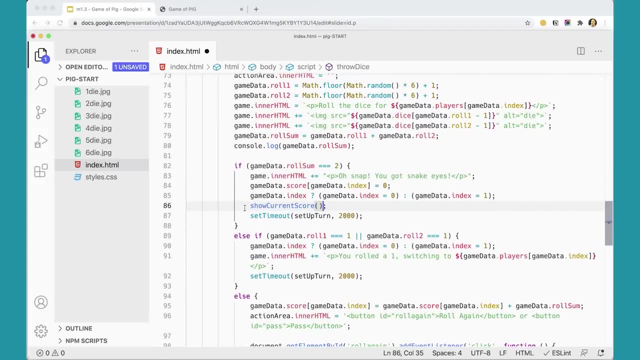 Um, so you could think about it that way. So there are lots of ways of doing things and there are lots of ways of thinking about it And um, and that's all really important. The the next thing to do is: 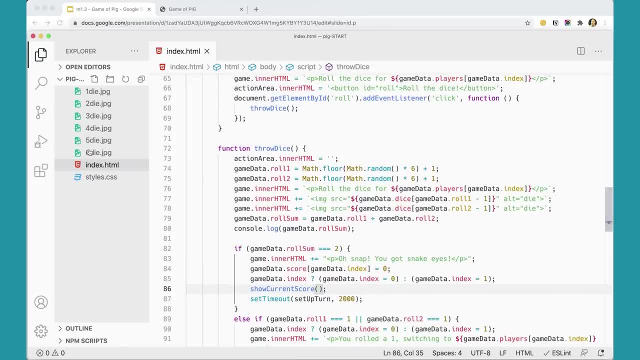 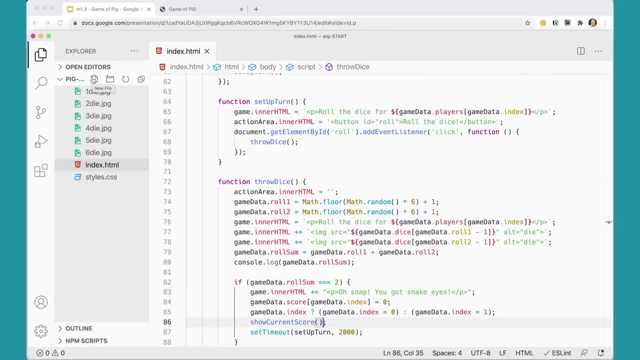 To apply some of our best practices to this, which would be to create a separate script file, is now. we've got a bunch of JavaScript at the bottom of the page. It's probably a good idea to make a new file here and call it scriptjs. 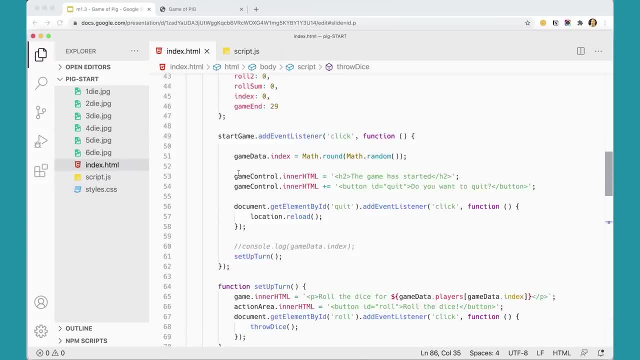 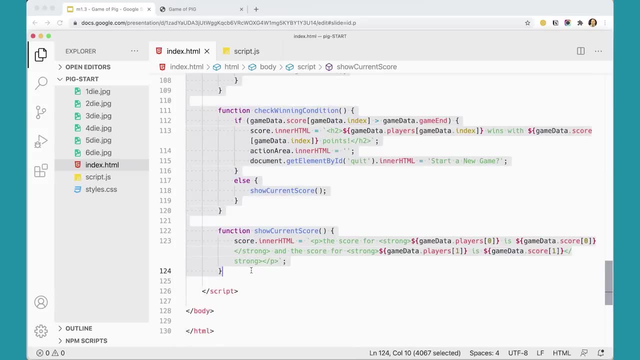 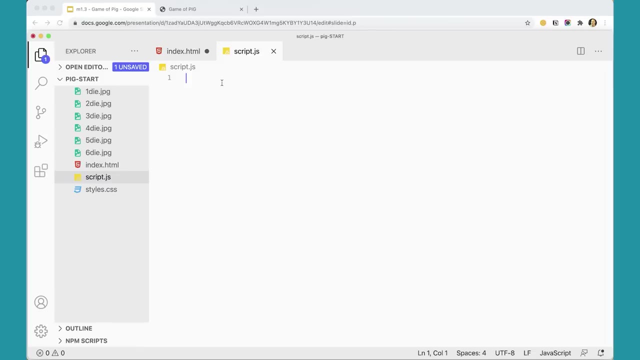 And on that file we could take all of our script from this, from the top here all the way down to the bottom of the script tag here, cut it and stick it on that script tag over there And in fact I'm going to put in my um immediately invoked function here. 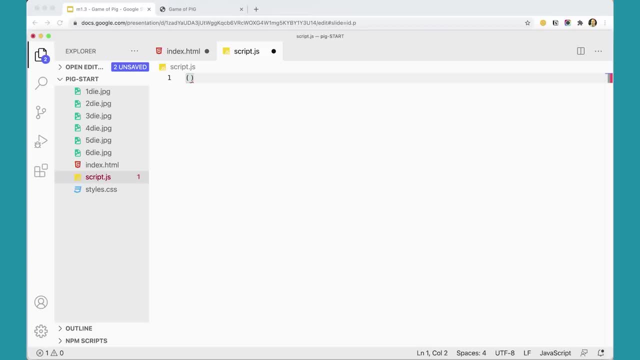 So I'm going to have parentheses and in there I'm going to run a function which has its own parentheses and its own curly braces and a set of parentheses after that and a semi-colon, And then I'm going to click between the curly braces and move that down and add my use strict. 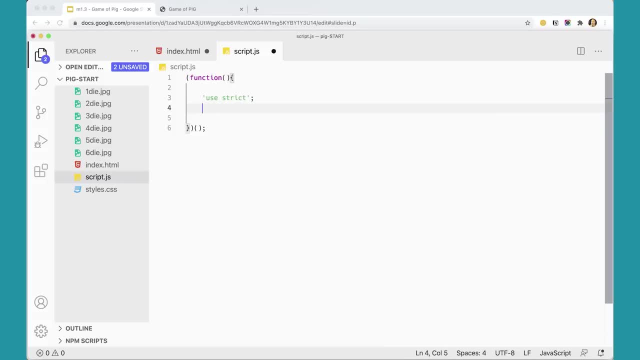 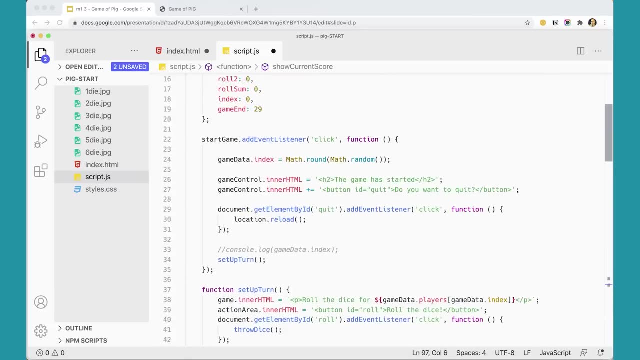 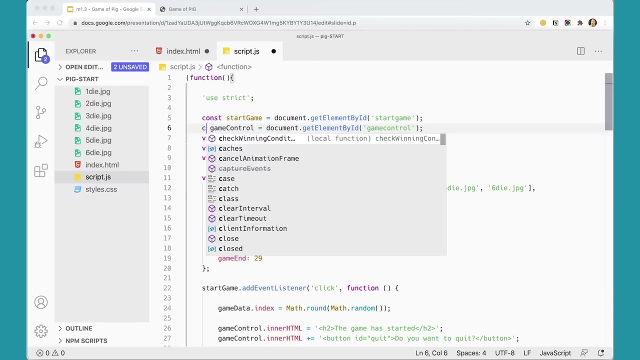 Directive to make sure I didn't screw up on any of my variables and then paste everything in So that puts everything in there, and then you could go through and you could change all of these two const, const, const, And in fact in this entire script all of the VAR declarations can be const. 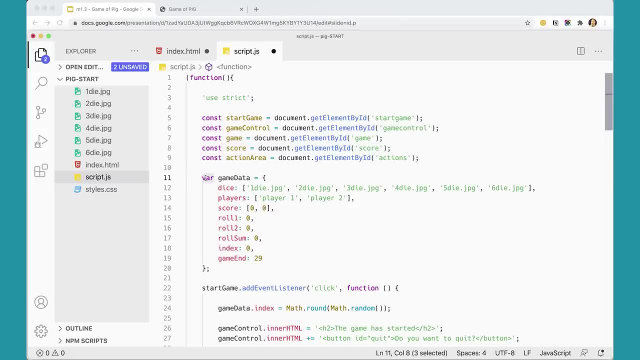 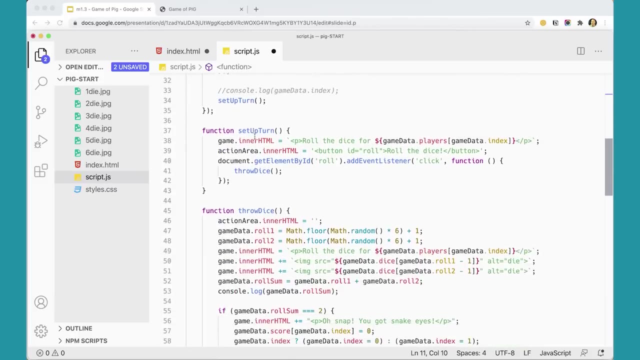 I think even the game data, Where the, the actual data changes, but this, the, the actual function, the, the actual variable doesn't change. So that can be const as well. Um, and then down here, do we have any other ones? 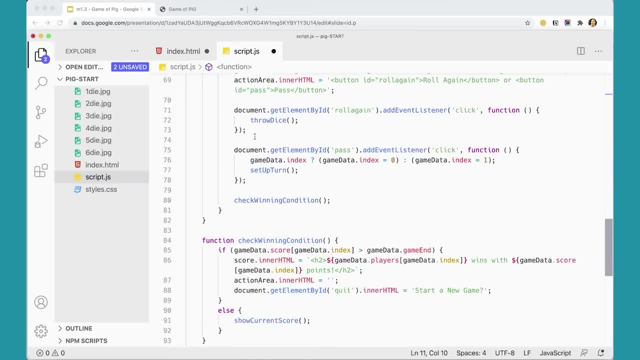 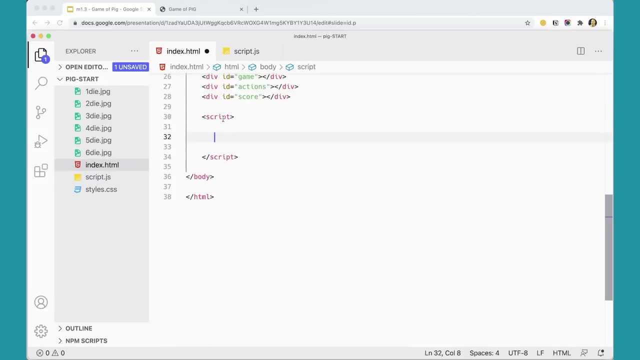 I think that might be all of them. Yeah, that's all. I think that should work. So we saved that and then we come over here and we move this up And we're going to link to SRC equals quote: script dot JS. oops, script dot JS. 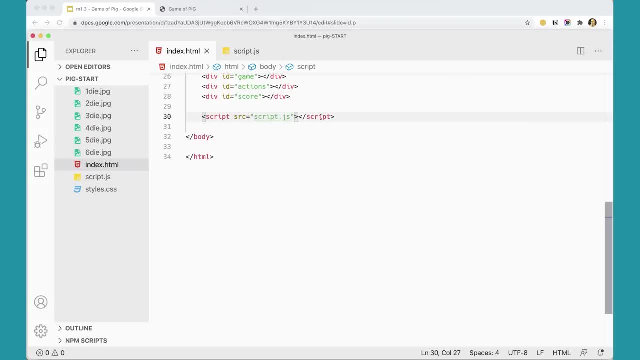 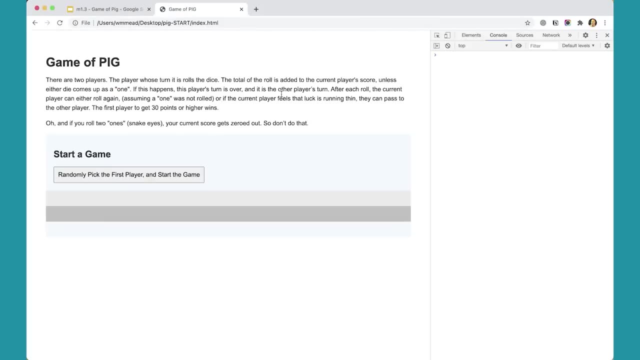 There we go, And you could move this up to the top of the page with a with a defer attribute on there as well. Let's just test this to make sure I didn't screw anything up. It looks like everything's going to work. 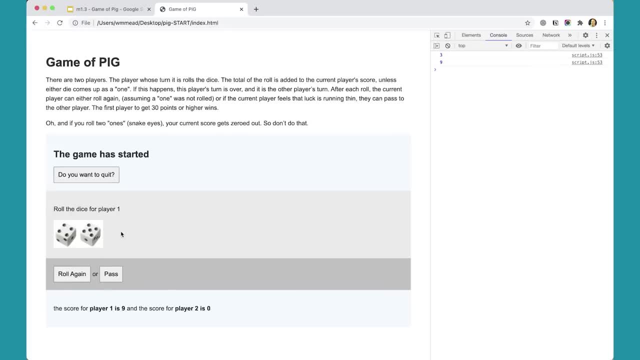 It's all working just fine. Excellent, So that's all working. That's good. So we've done. we've done that and that's important as well. Okay, great, So we've done all of the cleanup stuff. We have one last thing to talk about, but I'm going to do that in the next video. 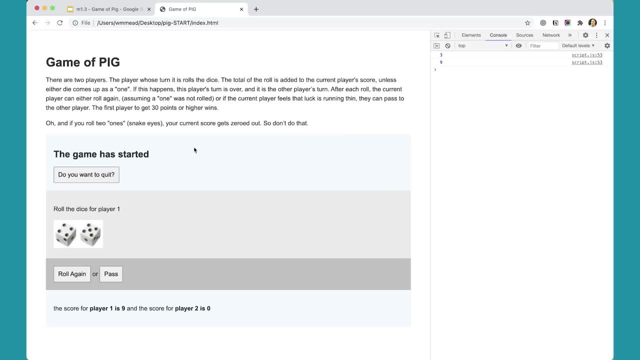 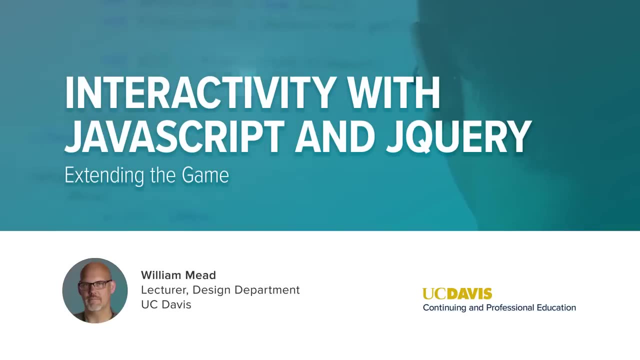 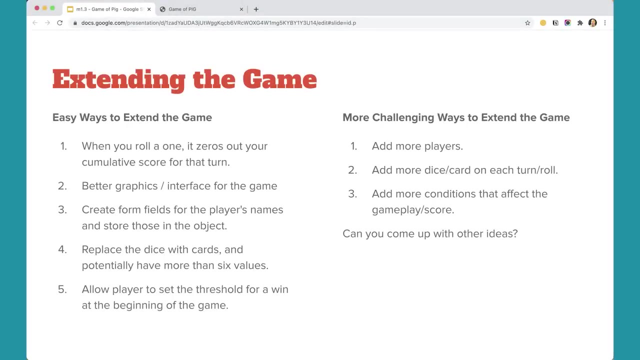 Um and um and you've got a working game here Extending the game. Okay, So now you have a pig dice game that works in functions, uh, and it's pretty basic. Um, and that's great, because we were able to plan and strategize a way of making a few different functions work together, to come together to make a game. 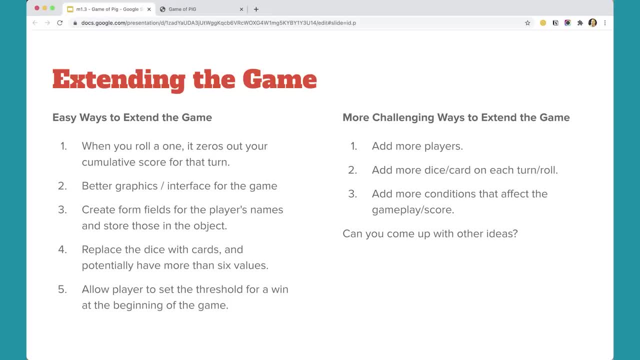 And that's definitely more complex than any of the scripts that we've done in the first course in the specialization, or the second course in the specialization. This is, you know, it's a good sort of medium place to be in terms of creating a more complicated script, but the game itself could be extended in lots of different ways. 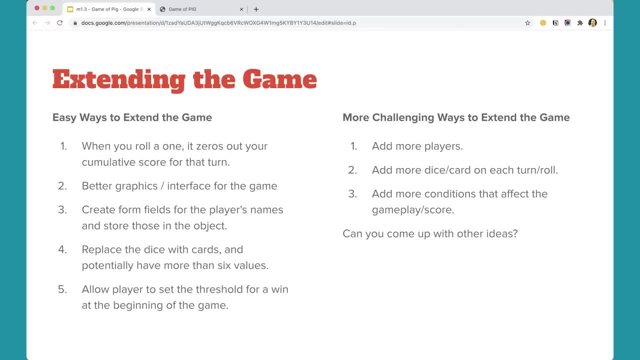 And my hope is that you will take this and run with it and do some interesting things with it, And I've given you some ideas for some things that you could do that are Not too hard and some that are more challenging if you really want to try to do them. 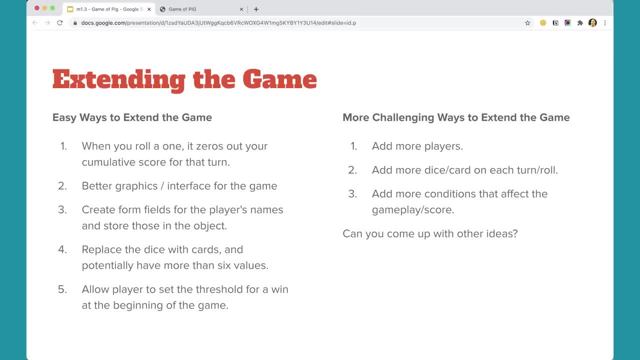 So the first is: when you roll a one, it zeros out the cumulative score for that turn. So if you think about this game the way it is now over here, when you play this game, there's no reason to ever click pass, really. 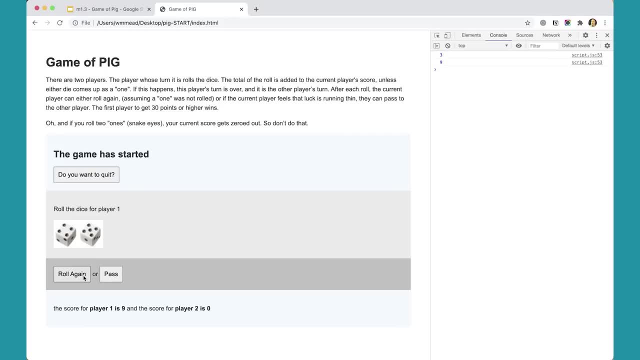 You're just going to roll again, and roll again, and roll again until you get a one. There's no strategic reason to ever click pass. But what if, If you roll a one, you lose all of the points that you gained during that turn? 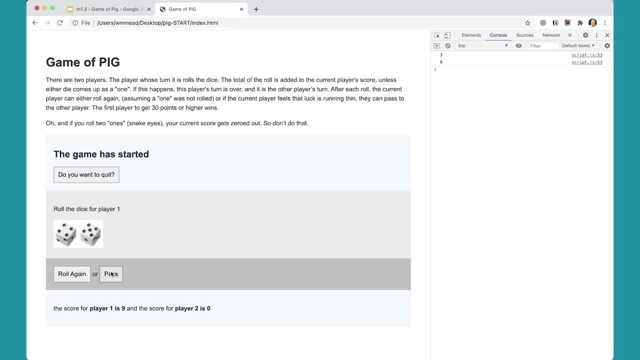 Remember, rolling two ones loses all the points you've got in the game so far, but rolling one one could lose all the points you've gained for that turn. So if you've got a couple of big rolls in there, you've rolled a nine, you've rolled a 12 or whatever. 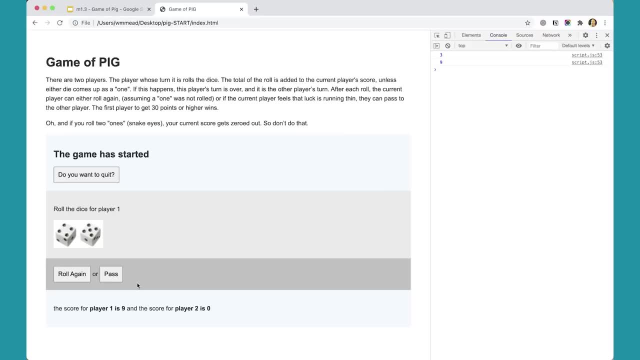 Now, pass could be, strategically, something that you want to do. Again, it's still just dumb luck as to what to do, Whether you're going to win or lose, but pass could be more strategic. So if you were going to do that, if you were going to add that feature into this game, what would you need to do? 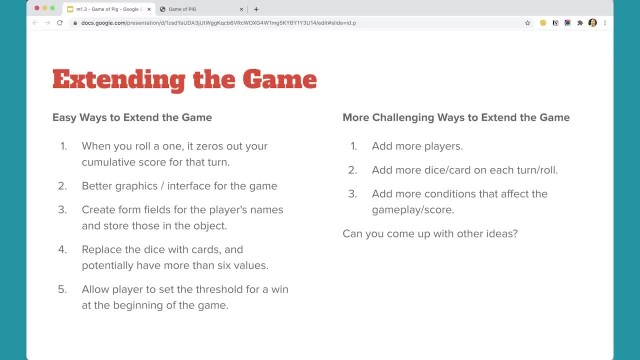 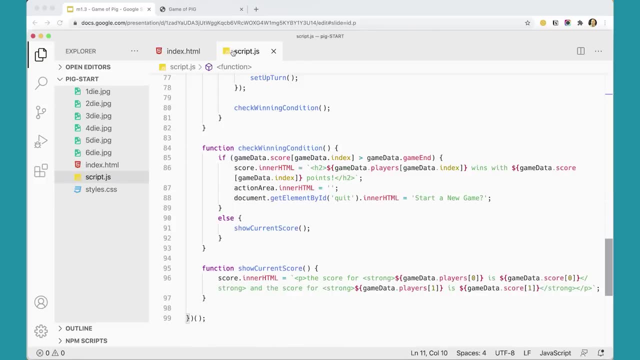 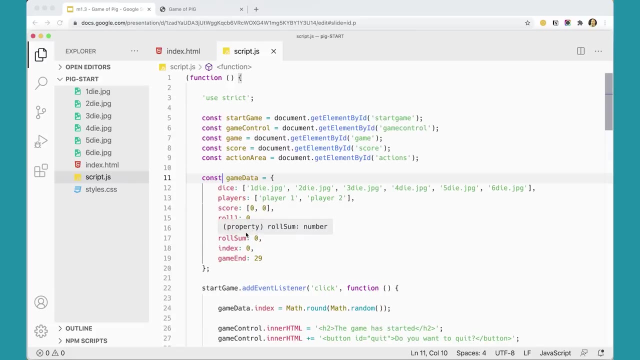 What would you need to add? I don't think it would be all that difficult. I think you could go back to your object up here and you could create another variable that says you know, turn sum or something like that, and each time a value gets added to the turn sum, you could increase that variable. 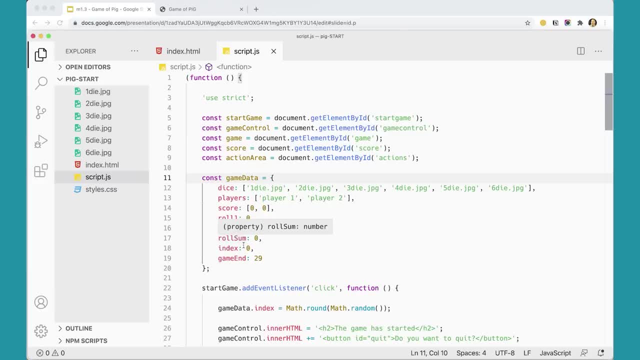 And if a one is rolled, you're going to subtract that from that player's score so that they lose those points for that turn. So just by adding one more property into game data you could add that feature in fairly easily. You just have to remember to update the rules. 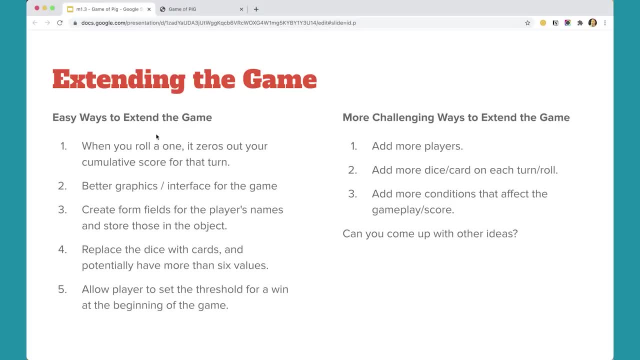 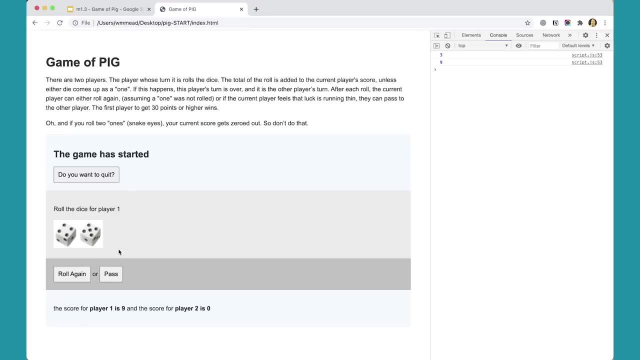 But that's just one way of updating this game. There are other easy ways You could make some better graphics or a better interface. make it look nicer, make it clearer whose turn it is and what the score is. None of this stuff is working terribly well over here for what I have so far. 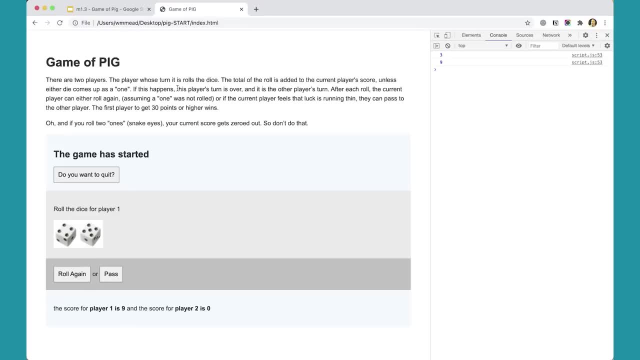 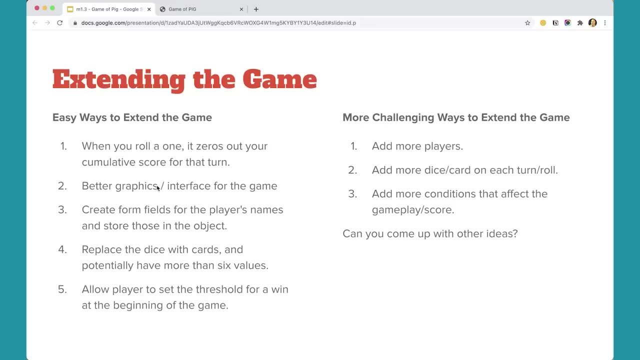 It's OK, but it's not. It's certainly not great. You can make it much better. So that's something you could do. That doesn't even involve a lot of programming, That's really just design work. You could create form fields for the player's name so that instead of player one and player two, 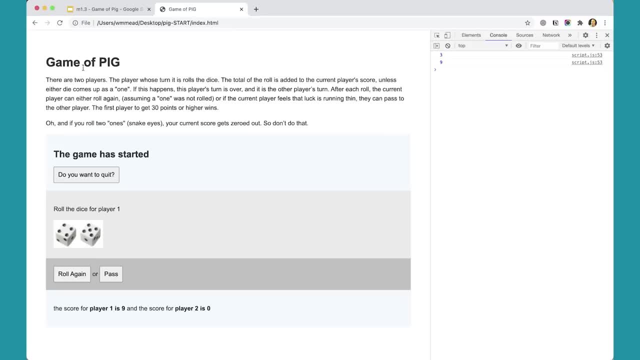 when you start the game, when you click start, you could, you know, instead of randomly pick a player you could actually enter in. you get up a form fields here, player one and player two. add those form fields in there. 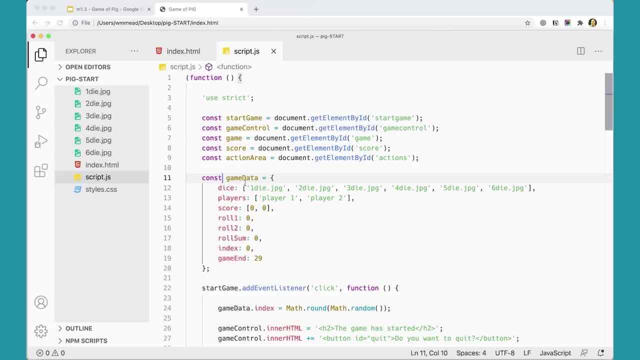 And again you would need to update your. you could replace these things here with the names that somebody types into the field so that it's not just player one and player two. So you could do that kind of thing. That would be more challenging but would be kind of a fun thing to do. 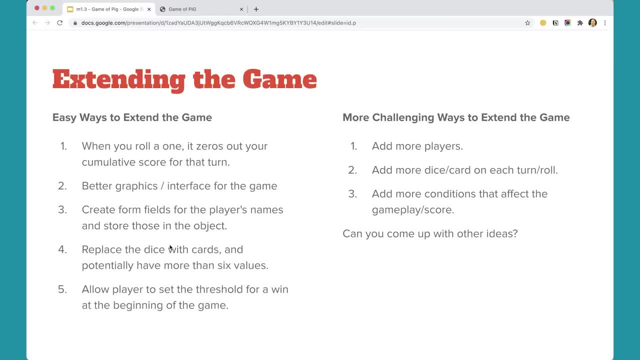 OK, you could replace the dice with cards. There's no reason why it has to be dice. You could make a cool card game. There's no reason that it has to be one to six. You could have 20 possible cards for each person and have more values. 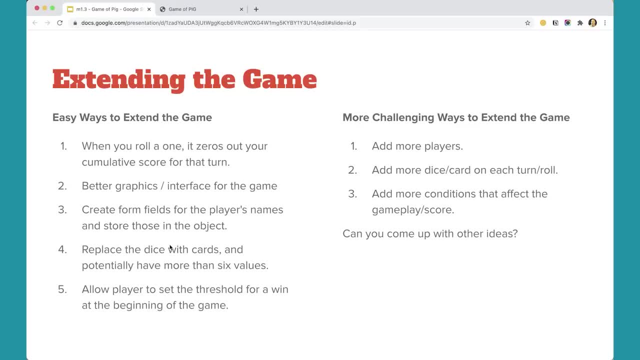 What would you need to change in order to do that? You could allow the player to set a threshold for what wins the game. Right now it's set to 30, which isn't very much, and you could just manually up it to 100. 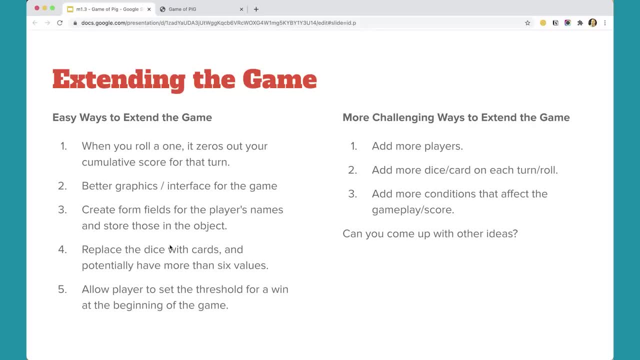 But what if, when you start the game, you have a field that says- or it could even be a drop down field for 30,, 50,, 100, whatever you want- And the player picks what the threshold for winning is going to be for that game? 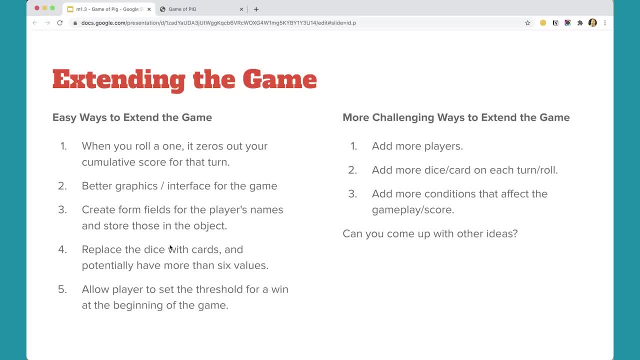 You could do that. That would be an easy thing to add into the game. And again, it's just updating the data in that game: data object at the top of the top of the game. OK, And then there's some more challenges. 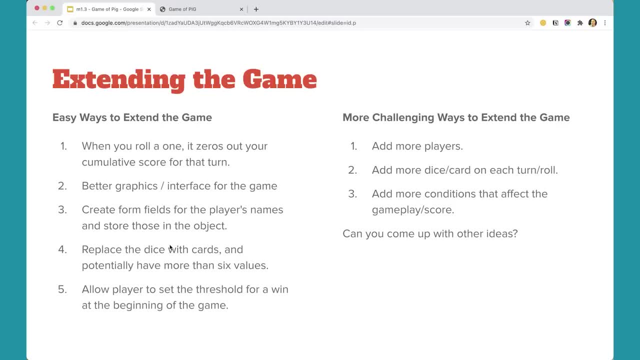 You could add more players. What if you had three players or four players? Or what if you could choose how many players you wanted to have playing the game? What would you have to add in order to do that? That's a bit more complex, because now that game index thing at the top of the page needs to be different. 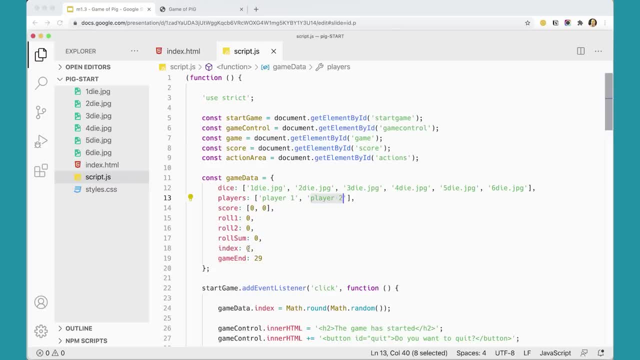 This needs to work differently, because it's not going to just be a zero or a one, And our ternary operators are no longer going to work because those will only handle two values, either a one or a zero. But you could certainly do it. 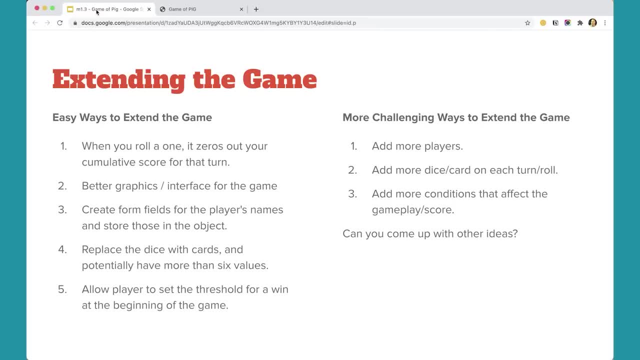 That wouldn't be that hard. That would be something more to do. You could add more dice. What if you had more than two dice? What if you had three or four? You could add other conditions that change that affect the game score. 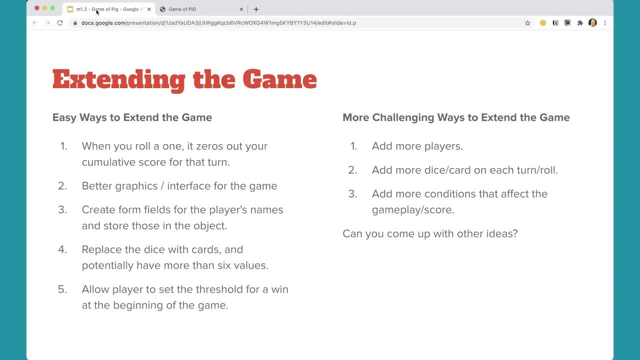 So what if somebody rolls two sixes? What happens then? Maybe their score doubles, I don't know. You could do all kinds of fun things with these, And there are lots of other ways that you could think of to come up with extending this game. 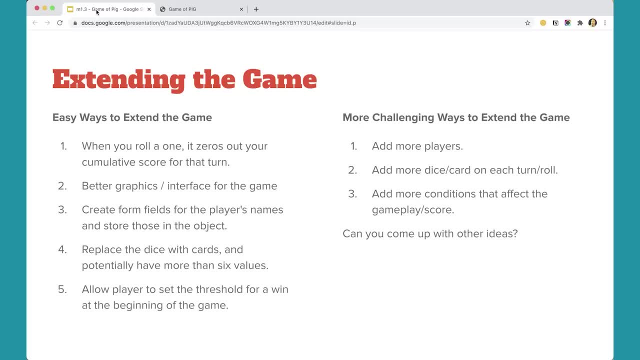 And that's your next job- is to really think about some things that you could do to extend this game and make it a more interesting, better game, And I look forward to seeing what people post on the discussion board. I'll check in from time to time and see what sort of excellent versions people have made of the pig game. 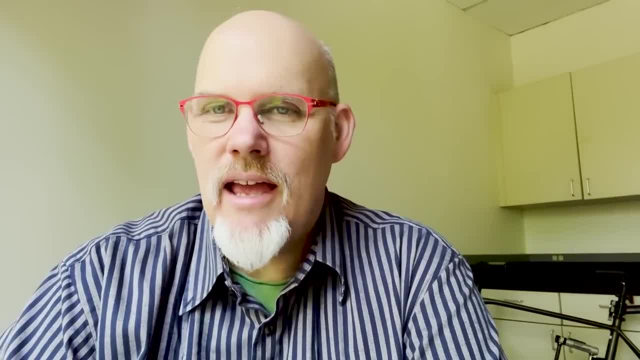 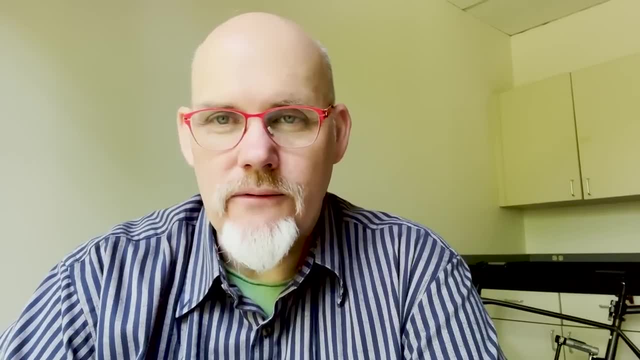 Congratulations for making it to the end of our third course on JavaScript in our four-course specialization. We've done a lot. You've learned a lot of JavaScript so far. In the first course we covered a lot of basics, a lot of basic syntax. 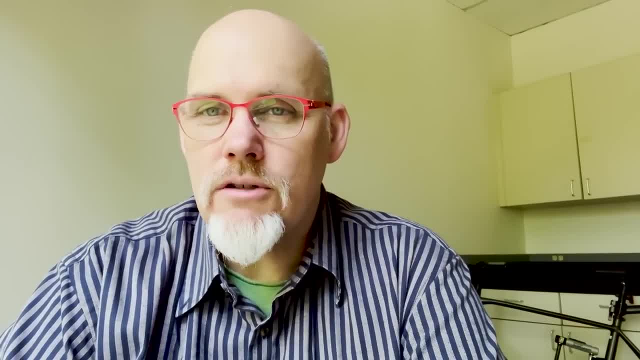 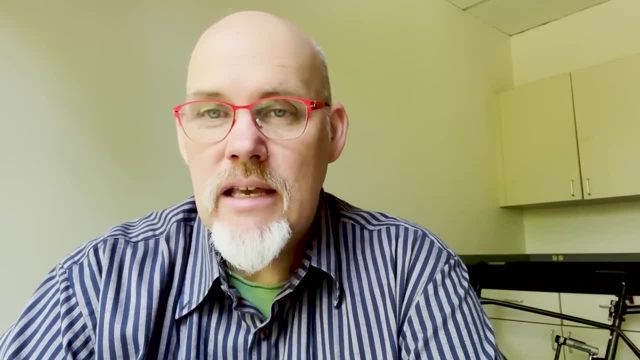 You did a lot of challenges to get good at that syntax. In the second course we introduced jQuery and we created some great interface elements that are very simple and easy to integrate into web pages. In this course we've gotten even deeper into it with jQuery plugins. 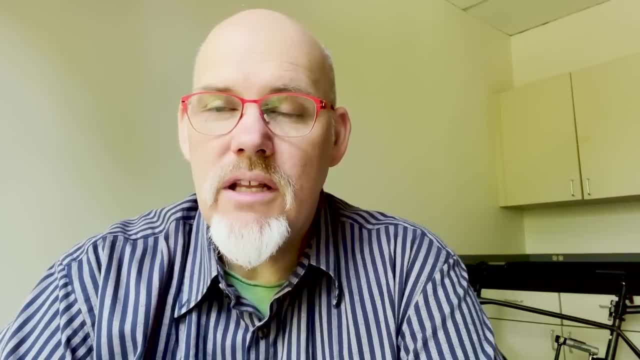 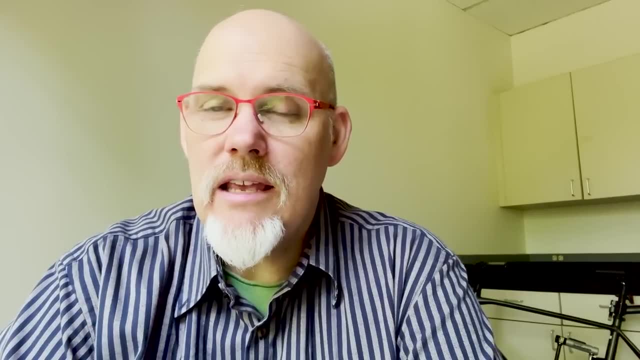 And you even created a game. So with all of this you've really developed a lot of JavaScript skills so far. We have a fourth course in the specialization And in that course we'll get even more complex scripts And I promise you're going to learn even more JavaScript and you'll get even better at it. 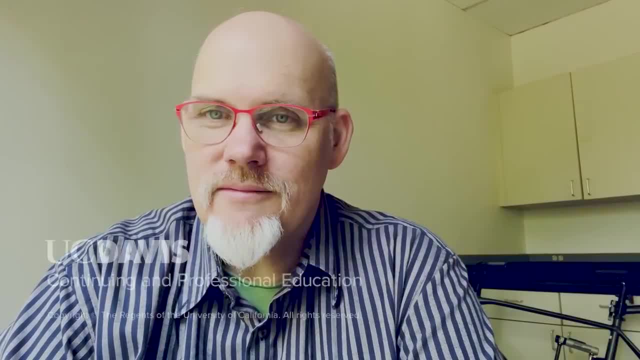 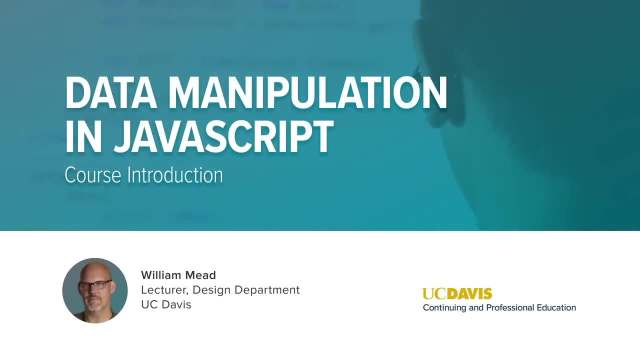 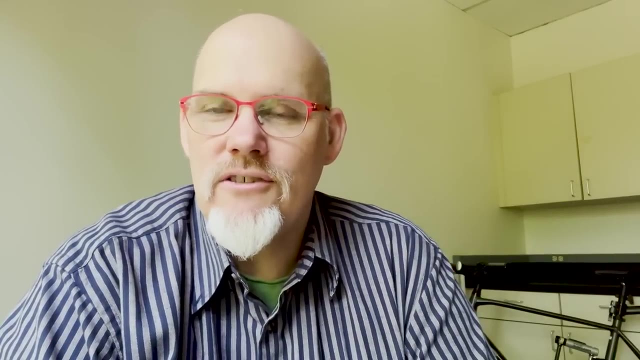 And you'll get more practice. So I look forward to seeing you there. Hello And welcome back. And welcome back And welcome to our fourth course in our four-course specialization in JavaScript. Congratulations for making it this far. My name is Bill Mead and I'm back to do more JavaScript with you. 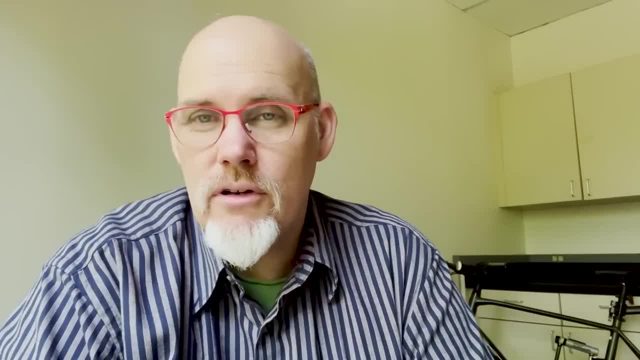 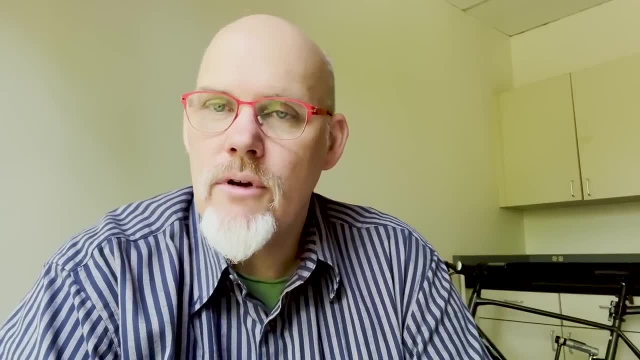 I hope you've had a lot of fun learning in our first, second and third courses. The first course we covered a lot of basics. The second course we introduced jQuery and compared that with JavaScript. In our third course we got more deeply into JavaScript and created some more sophisticated scripts. 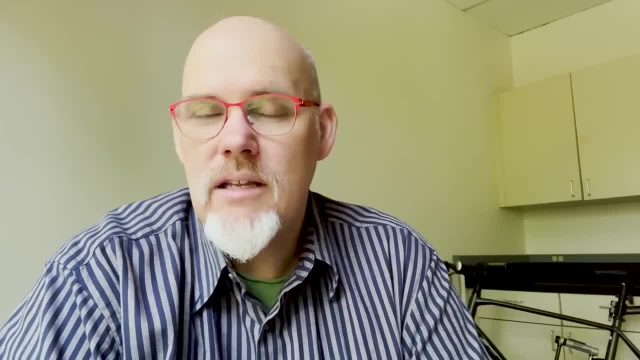 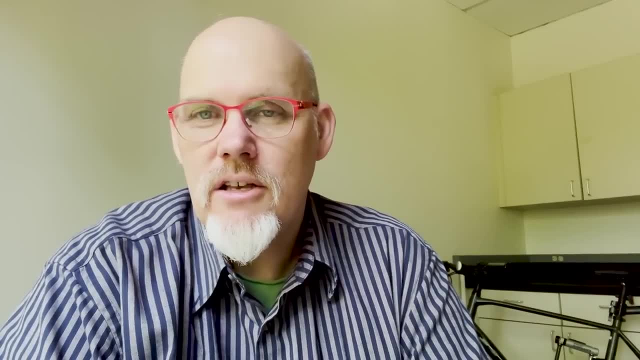 This course we're going to take it even further and you'll learn more In-depth JavaScript. You'll learn some more skills and techniques, You'll get lots of practice And I promise you'll get a lot out of it. So join me for this final course in our four-course specialization. 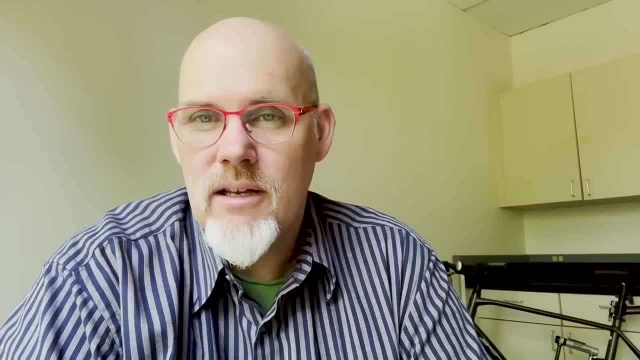 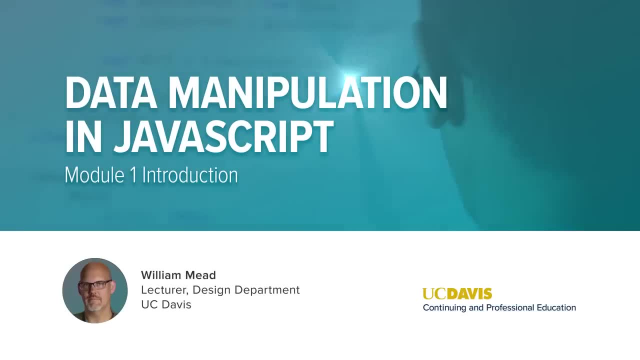 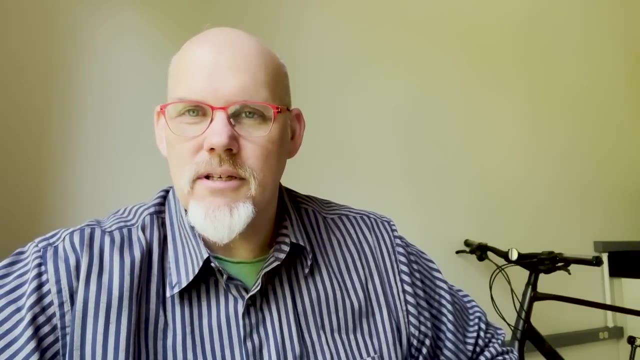 And I look forward to working through this material with you. I think you're going to have some fun with it. Hello And welcome to the first module in our fourth course on JavaScript. In this module, we'll look at some of the things that we've learned about JavaScript. 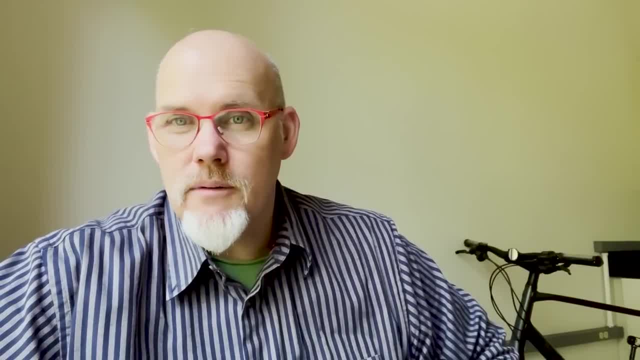 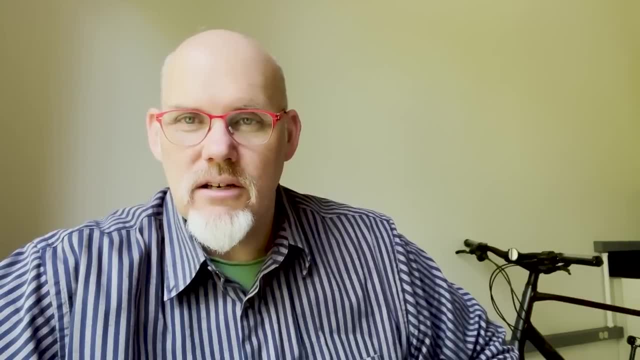 We'll look at forms in HTML and how to get data out of forms and process it and validate it. This is a vital thing to know And it's really important that you learn these skills and these techniques. Plus, there's lots of great practice and you'll gain a lot of skill along the way. 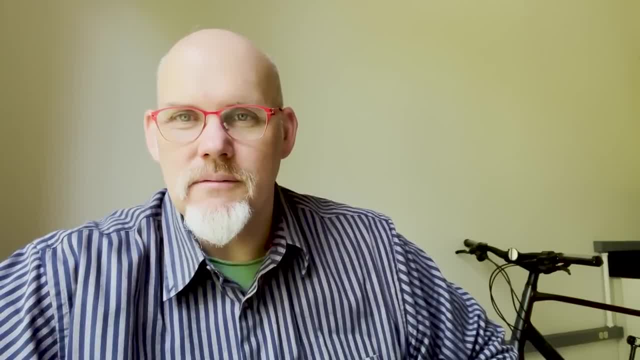 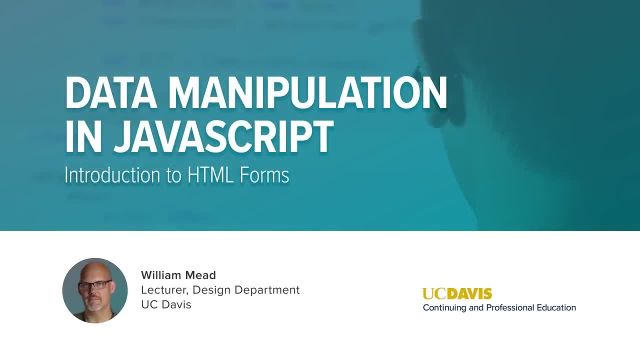 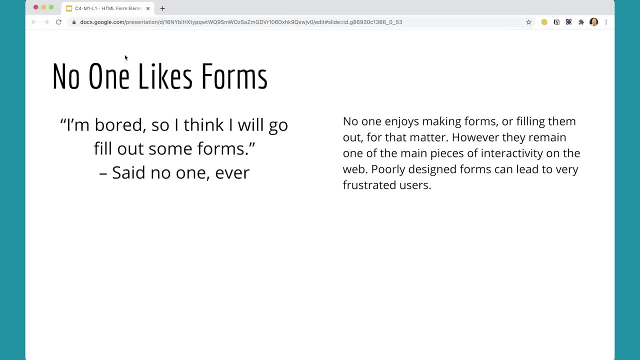 So let's get started And I look forward to working through this material with you. Basic HTML- HTML form elements. No one likes forms. I'm bored, so I think I'll go fill out some forms said no one, ever. No one enjoys making forms, or filling them out, for that matter. 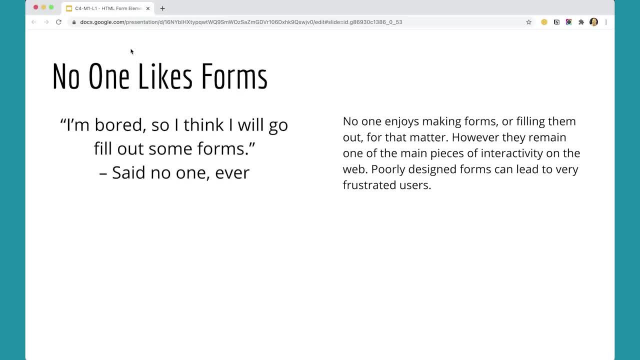 But they do remain one of the main pieces of interactivity on the web or in digital products of any sort. It's one of the main ways that we collect data from users, And poorly designed forms can lead to very frustrated users. If you've had to fill out a form, it's going to be very frustrating. 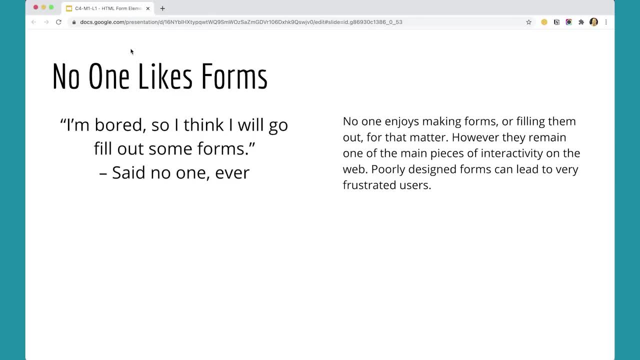 If you've had to fill out a job application recently, you've probably come across a poorly designed form. They can be very frustrating And if people don't take care to design them properly, then it becomes much, much worse. And as we go forward in this course, 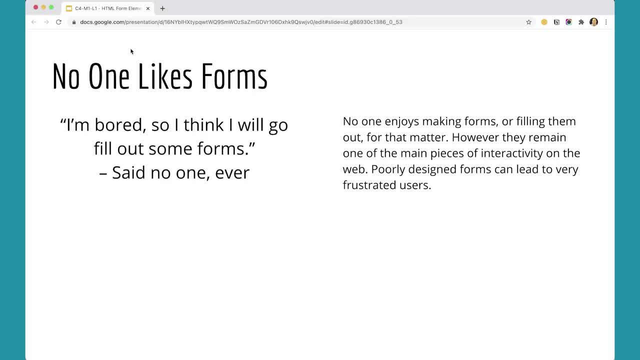 we'll be looking at how we can collect data from users and what we can do to make sure that we're getting the correct data from users, and looking at ways in which we can improve the user experience by designing forms properly. So let's get started with that. 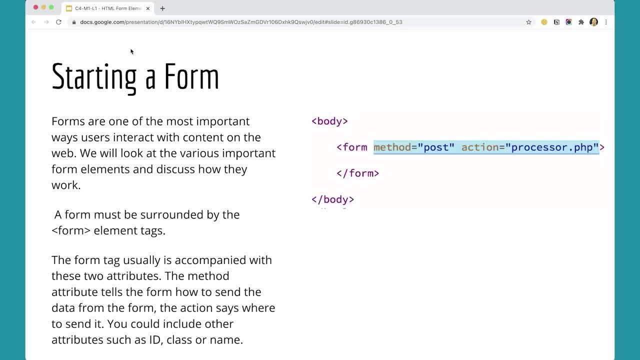 To start a form, we would start with a form element in HTML, And usually there are two attributes that go with the form element. One is the method which would either be set to post or get generally, And that has to do with how the data is sent. 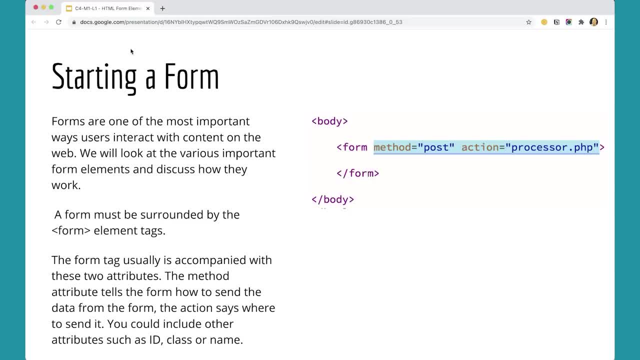 And we'll explore that more later, exactly what that means. And then the action is the file that the form data is going to be sent to. It could be a PHP file, like I have processorphp here. That file isn't going to exist in our project. 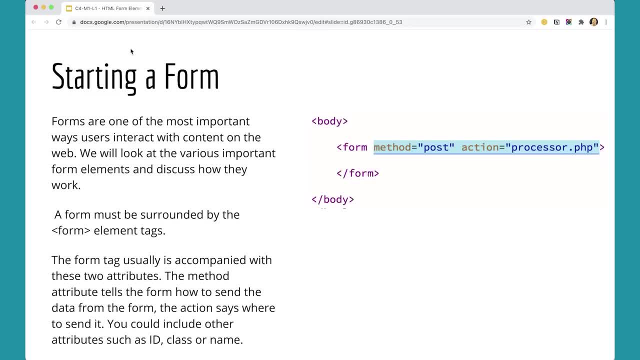 but that would be where the browser would think: okay, when somebody submits this form, that's where it's going to go And we're going to send the form data to processorphp. So it could be a PHP file, It could be. 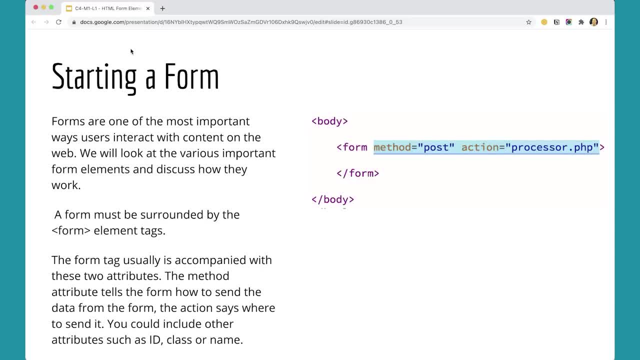 A Perl file, It could be any sort of server-side file that's going to take that data and then do something with it, like send it in an email to somebody or put it in a database or process it in some other way. So those are the basics. 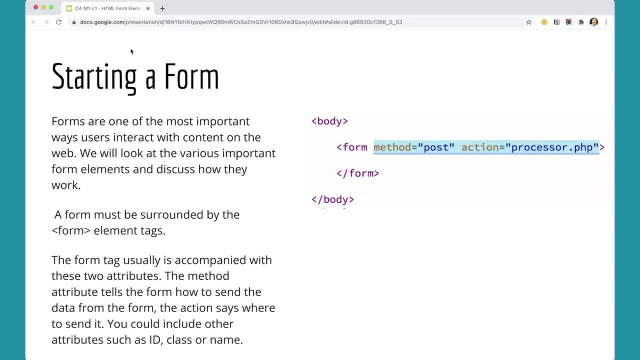 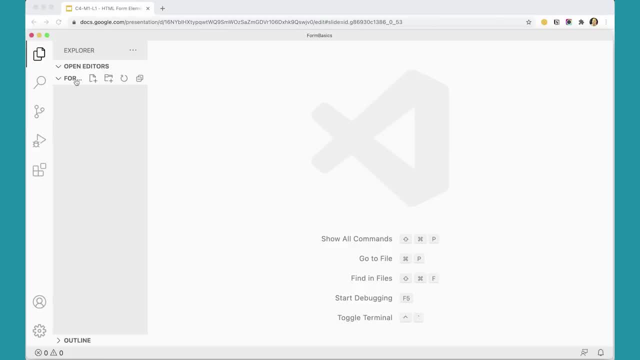 And what I recommend you do is just make a folder on your desktop, a directory in your desktop, and open it up in Visual Studio Code. I have a directory called Form Basics that I created And I'm going to make a file in it called indexhtml. 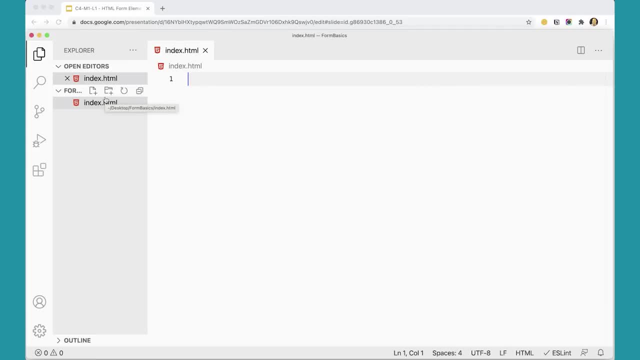 And just to get used to creating these basic form elements. I'm going to just create a basic form here. It's not going to have a lot of styling, but we can see exactly how these elements get rendered with the default styling in our web browser. 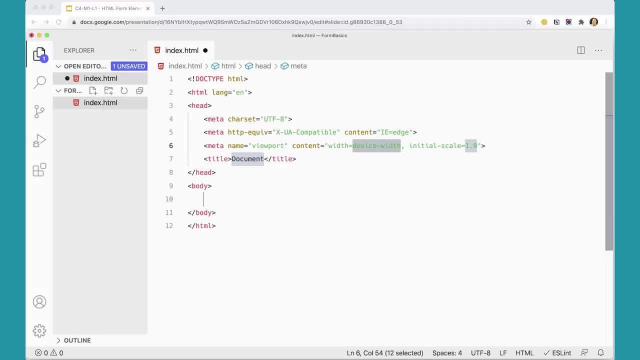 So, to get started, I'm going to use an exclamation point and press tab to generate my starting HTML. here I'm going to just call this form basics And then down here I'm just going to add maybe an h1 form basics. 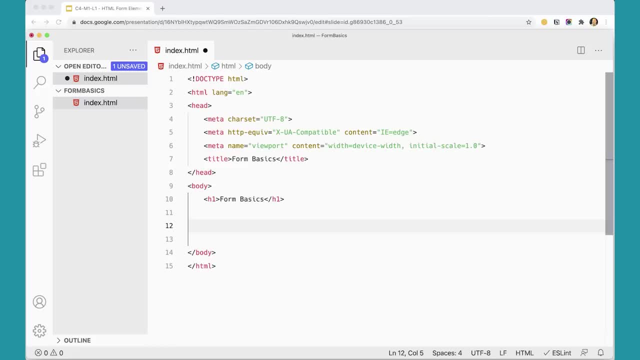 And then I'm going to add a form tag form And it opens and closes And I'm going to set the method And then I'm going to add a form tag to post. Now it doesn't matter what order these attributes go in. 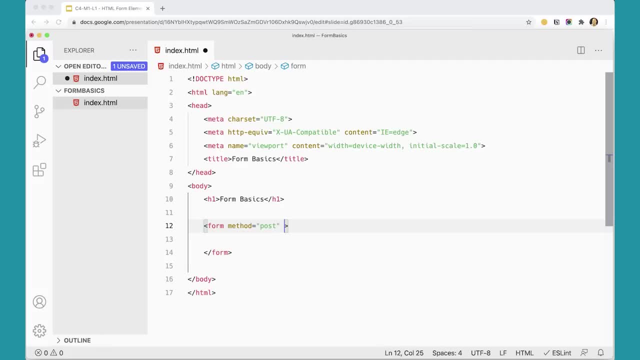 You could set the method first or the action first, or you can be. You know we're not going to actually process these forms. You could leave off the action altogether, But I'm going to put it in equals processorphp, something like that. 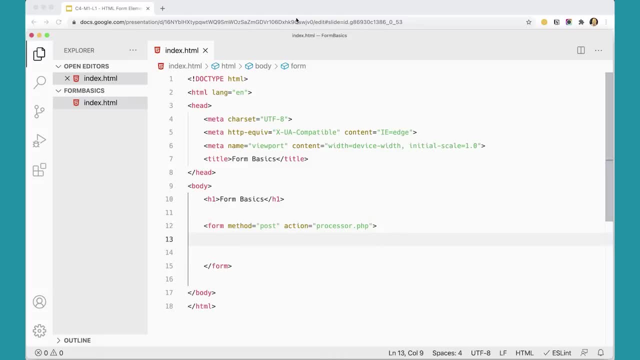 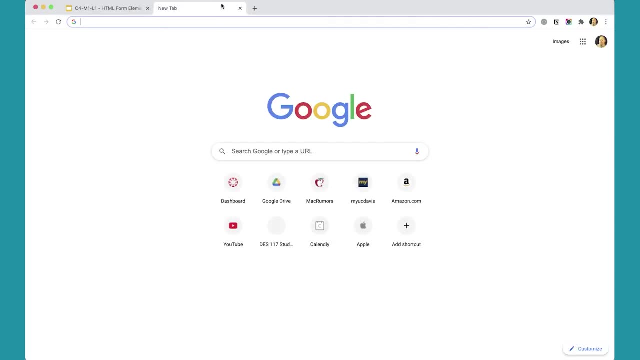 OK, so now I have the start of a form element on my page. Come over to here and just open a new tab and open this up in my tab here. OK, so I've opened up my indexhtml, which just says form basics. 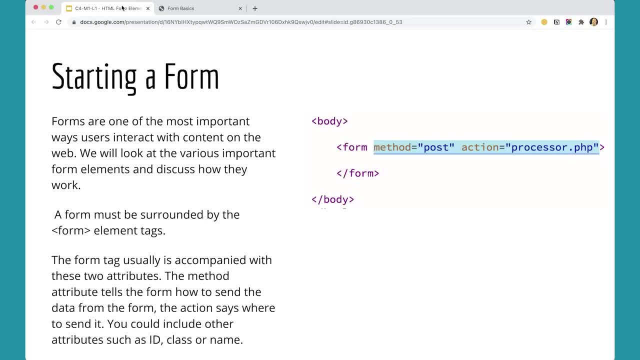 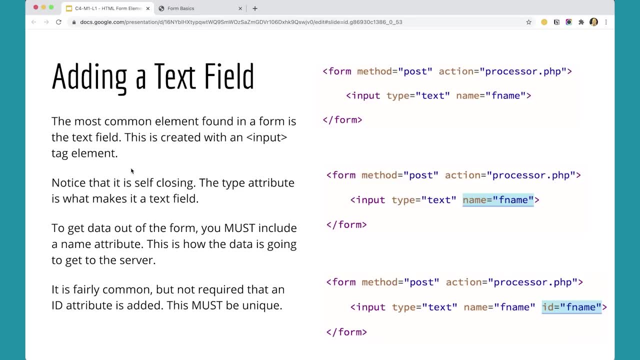 There's a form here, but there's nothing in it, so it doesn't show anything. All right, great From there, let's move forward and see what we can do with this. First, I'm going to add a text field for someone's first name. 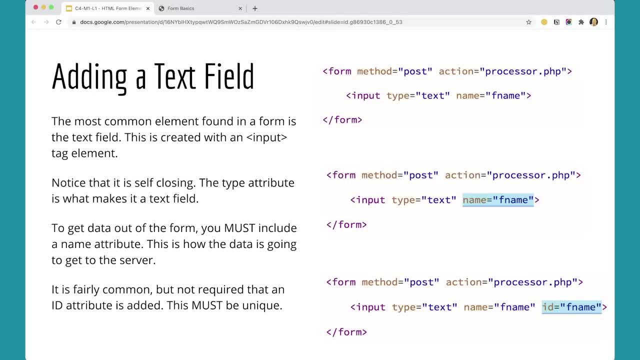 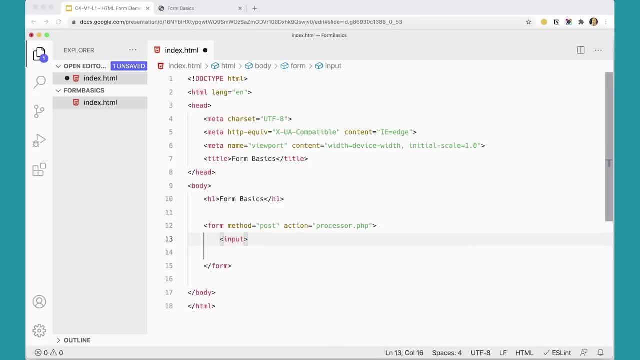 So let's take a look at how we do that. I'm going to add an input and the input element is self-closing, So there's no closing one with a slash, It's self-closing. And I need to add a type attribute because there are a number of different types of inputs. 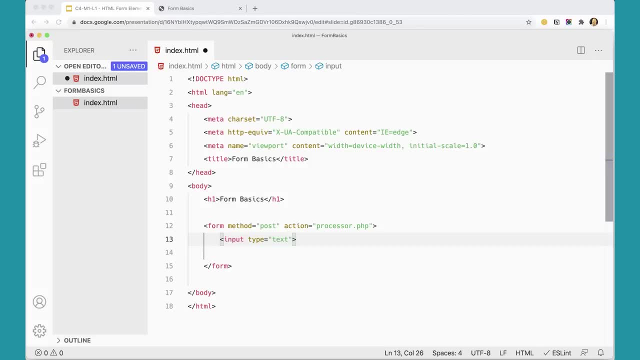 Let me just start with text, just the most basic input, text input. And then you could add an ID Fname. for first name You could add a name attribute fname. The name attribute is important if you're sending the form data to a file like processorphp. 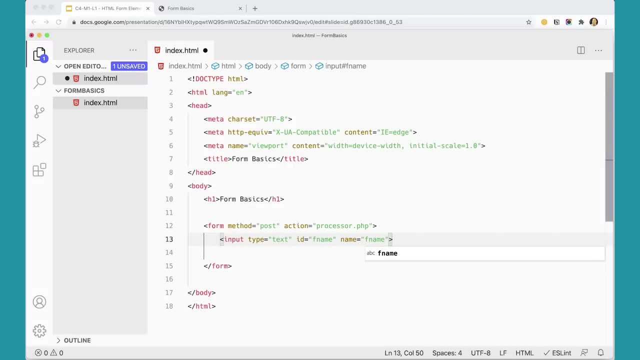 that's going to process the file, process the form, because the way this processorphp would recognize this data is through the name attribute. So even though these two things have the same value in them, they serve different functions. This one gives this particular field or input an ID that I can target specifically with JavaScript. 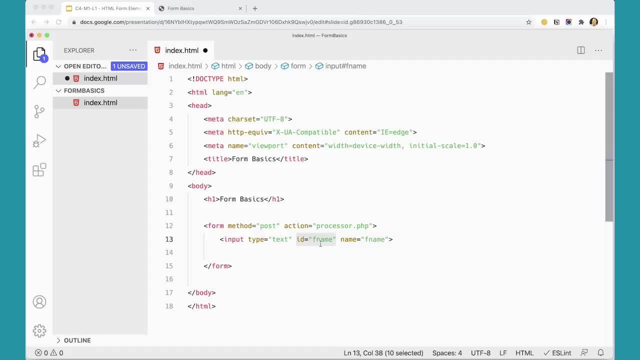 And with JavaScript, that kind of thing, And this one is something that I would need when the data gets sent through. These are the basic. These are the basic attributes that I need, but there are other attributes you could add. You could add a value. 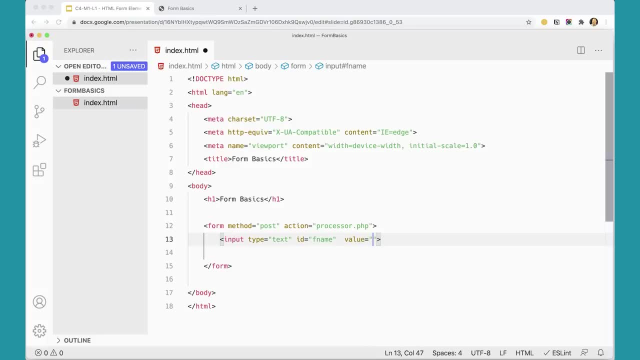 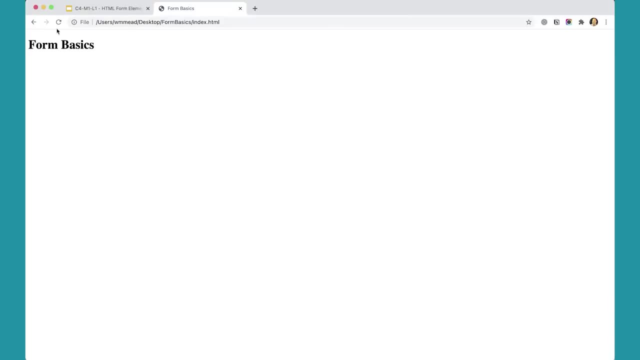 That will show up as a default value in that field. If I come back over here and refresh this, you'll see it will show up as default as a default value. in there You could add a tab order. So if you have your field set up, arranged in a certain way, 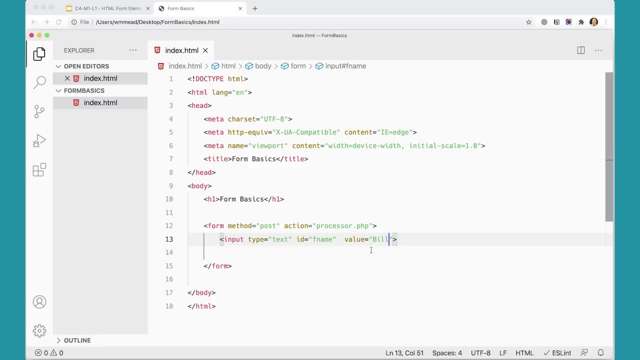 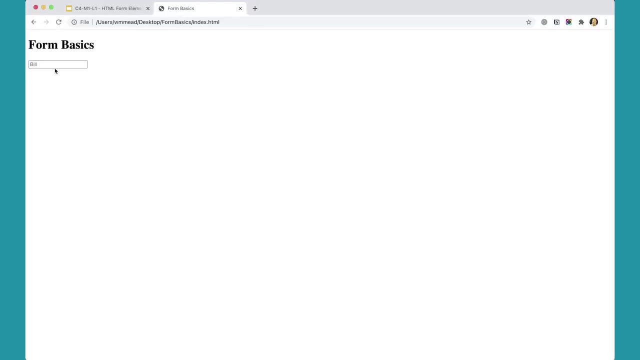 way and you want people to be able to tab them, tab through them in a certain way. you could add tab order, something like that, but you can add placeholder. the difference between placeholder and um value is that placeholder will simply put in some text. as soon as i click in there, i can start typing something else. 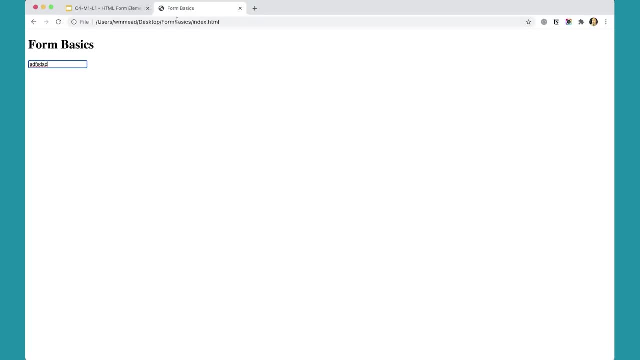 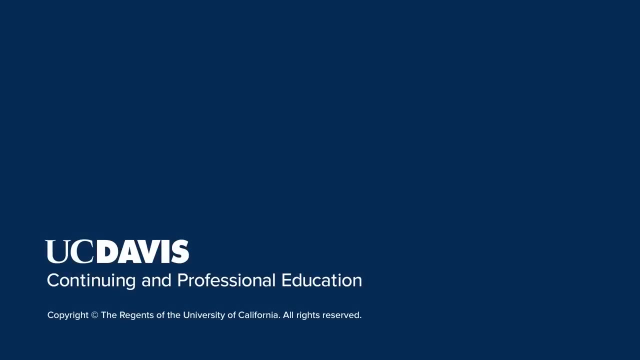 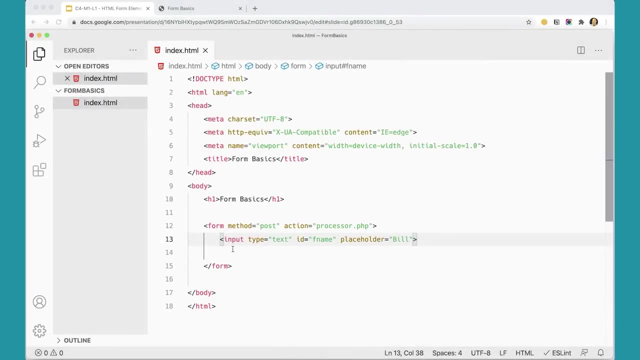 where it's not actual content of the field. so these are some of the different actual content of the field. so these are some of the different different pictures and pictures that i could type in there- attributes you could put in there. We got our form started and we've added an input field of type text with an ID and a. 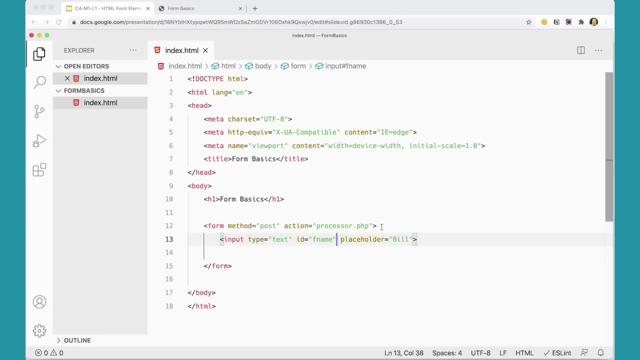 placeholder here. Now we could also add a label, and labels are how people know what sort of data is supposed to go in each field. So we'd use the label element like so: first name: The label element gets a for attribute. for equals quote: fname. 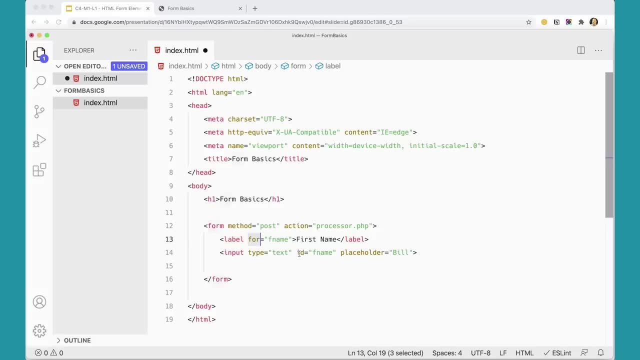 Now this for attribute connects very directly with the ID so that our browser knows this label. It goes with this field and it connects to the ID. We might also have a name attribute of fname. That may be important for us, but specifically, and these may have the same value in here: 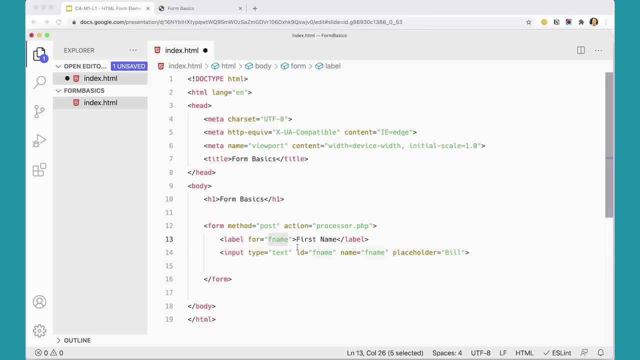 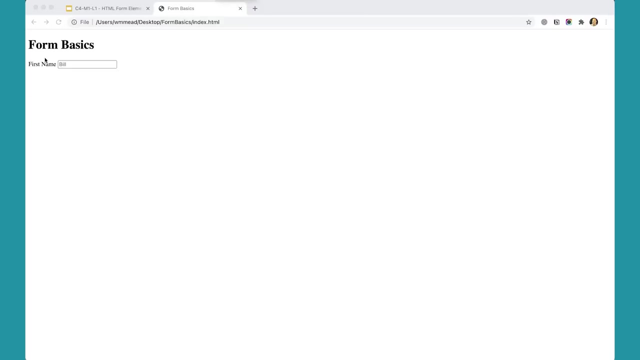 but specifically this attribute is talking specifically to this attribute. They're connected to each other. In fact, we can test this over here. Here I am on my form. If I click on the words first name here, you'll notice that it puts me right into that field. 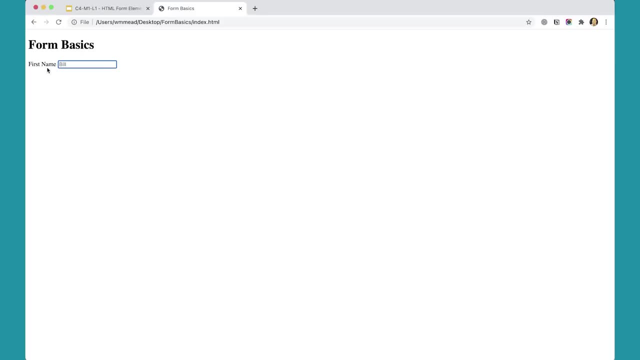 And that's because by clicking on the label, it knows the label is connected to the field. So that's kind of that's actually an important usability feature. Later we'll talk about checkboxes And rather than having to be in the field, we're going to talk about checkboxes. 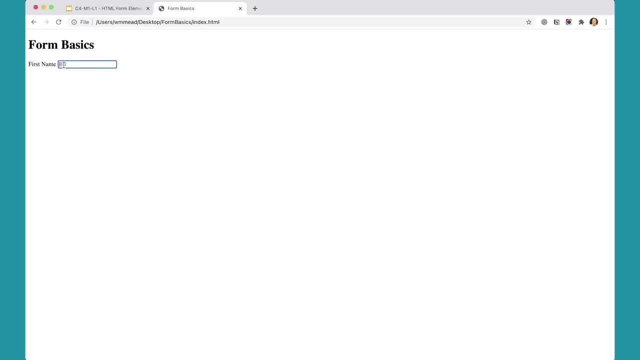 And rather than having to be in the field- we're going to talk about checkboxes- And rather than having to be a surgeon with your mouse to be able to get in into a field, you can just click on the label and it'll put your cursor in that field. 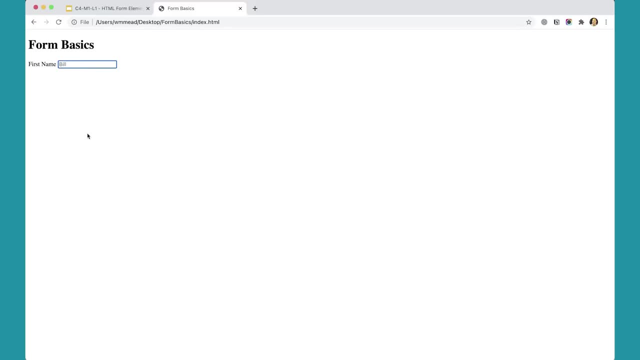 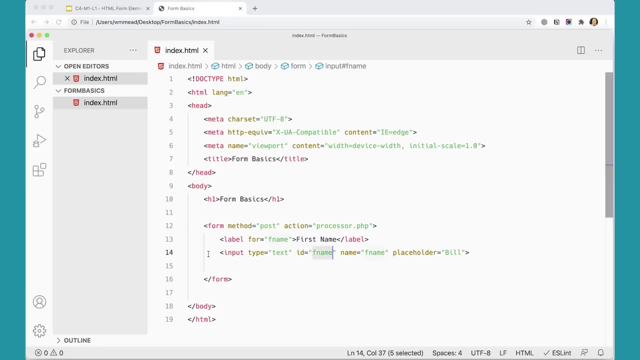 Or if it's a checkbox or radio button, it'll actually check it. We'll look at those in a few minutes here. So that's one way of working with labels. There's an alternative syntax to labels, which is you can not use the attribute and instead 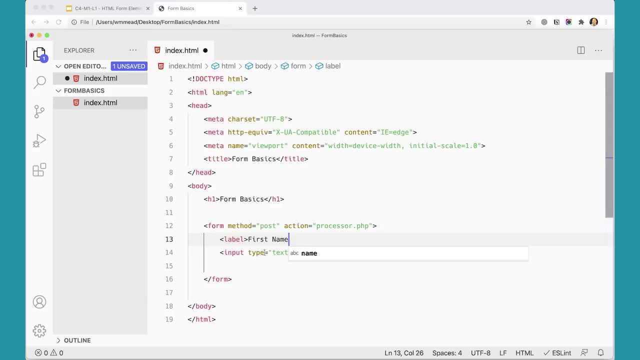 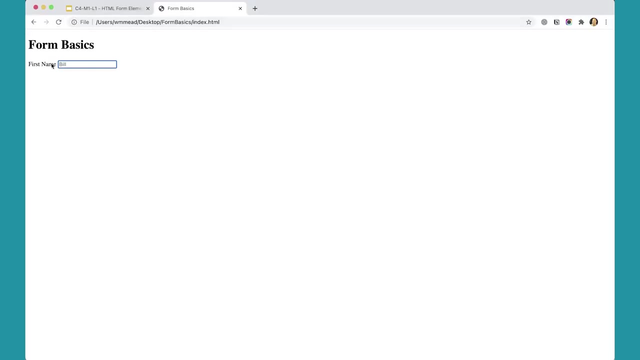 surround the entire text input with the label tag, so that the input tag is inside the label. This will also work. This is valid HTML, So you can do it this way as well. If you refresh over here and click on first name, you see it works. 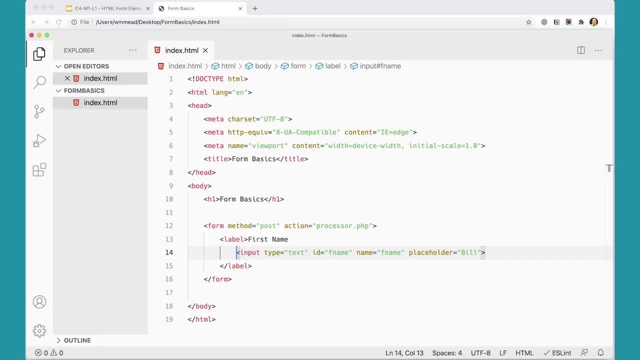 It goes in there, So that's fine. But you're more likely to see it the other way around, like this with the for attribute, partially because it makes it easier for styling if these two elements are separate. If you wrap it inside the label then it can be a little bit more work to get the styling. 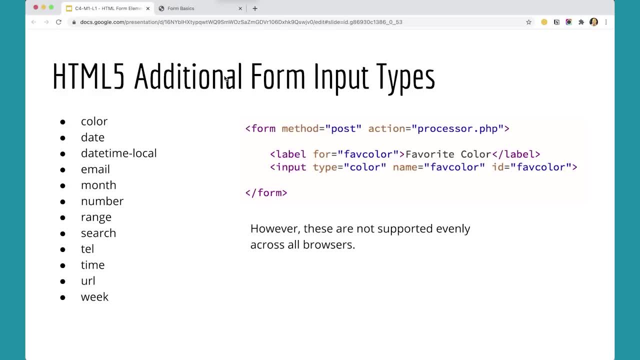 to work the way you want it to work. There are a number of different HTML5 form input types. So still using the input Element, here you could- actually we've used text, but you could do email or month or number range or tell or time or URL or week. 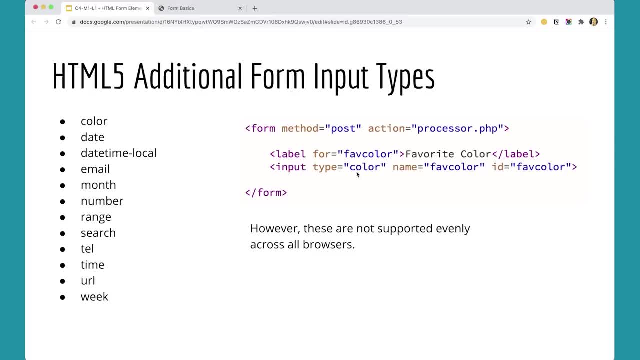 There are a number of different input types that you could use in place of text here. Here I'm showing the color one. Let's go ahead and give this a try, And not not all browsers will support these in the same way, but it's. it's worth trying. 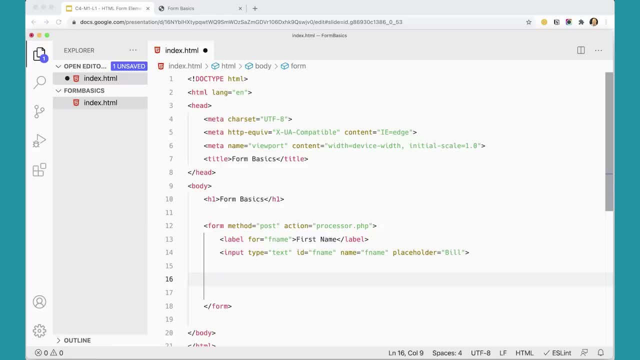 them out and or they might support them, but they might Style them differently. That's another thing that can sometimes happen. So I'm going to have label for fave color, favorite color, and then I'm going to have an input. 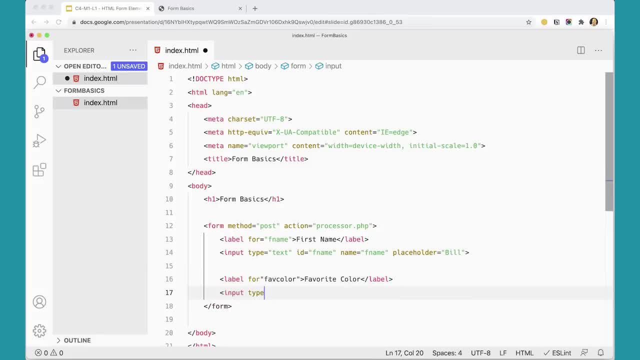 Input type equals color, And then I'm going to have an input Input type equals color, And then I'm going to have an input Name equals fave color, And then, don't forget, the ID ID equals fave color, like that. 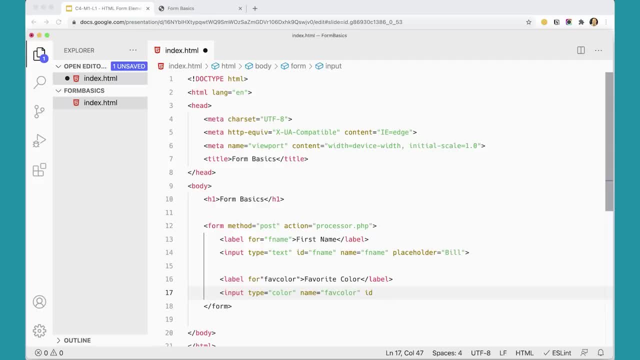 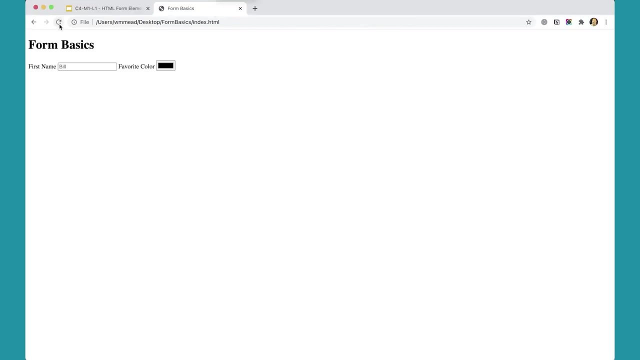 Now let's go back and see how that gets rendered. So now I have favorite color, I click on this thing and it gives me this interface element here, And this is being provided by the browser, So this might look different in a different browser. here I'm using Chrome, but it might. 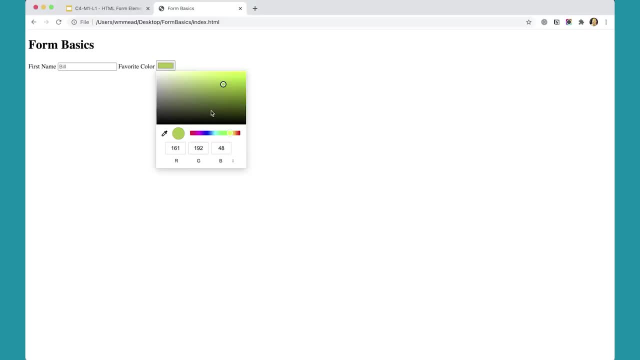 look different in Firefox or Safari or Edge or some other browser, depending on how the browser is set up. The other thing to notice is that, by default, labels and input elements are inline elements, So these are lining up in a line And if you don't want them to line up in a line, if you want them to get stacked vertically, 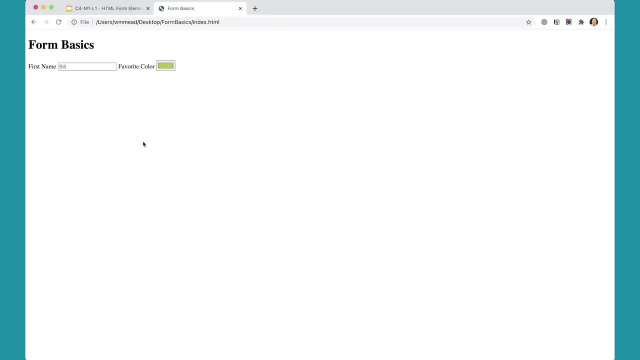 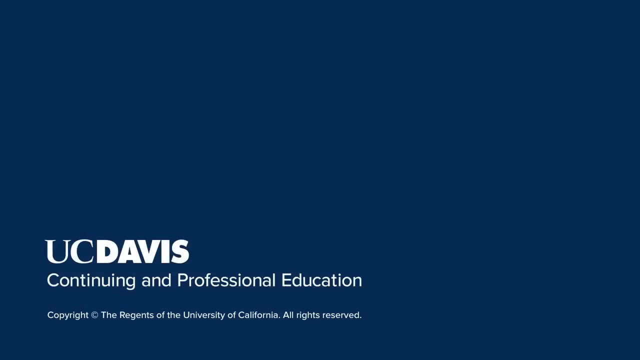 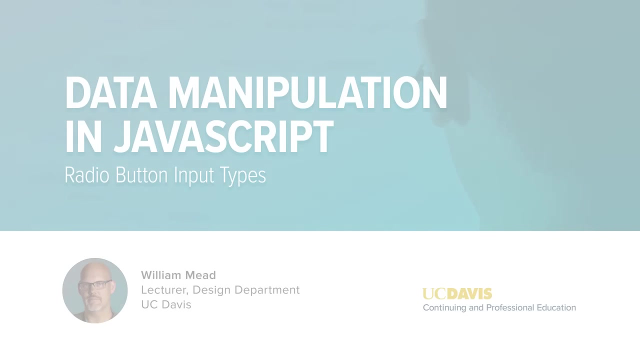 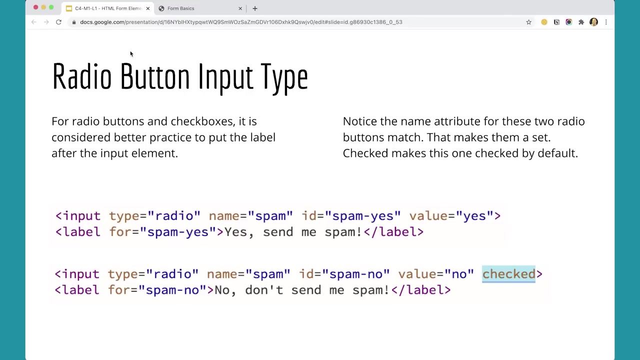 which often you do. you can set them in your style sheet to display block and then that will make them line up vertically. Let's talk about radio button input types. For radio buttons and checkboxes It's considered better practice to put the label after the input element. 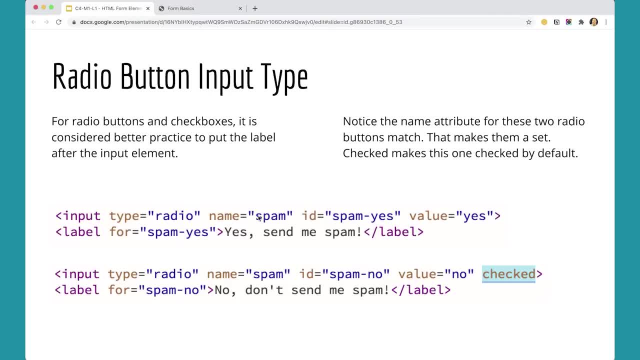 Notice the name attribute for the two radio buttons match Name spam, name spam. That puts them as a set so that only one of the two can be checked, And then the attribute down here, checked, makes this one checked by default. 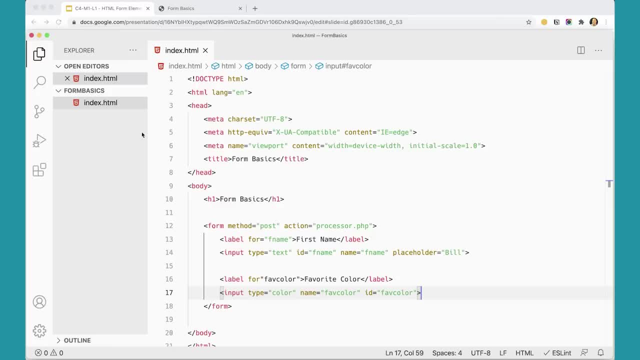 So let's go ahead and give this a try over on our code. just going to add these on in here. So input type equals radio, like that, and name equals spam and ID equals spam- yes, and value equals yes. You have to add a value on these. 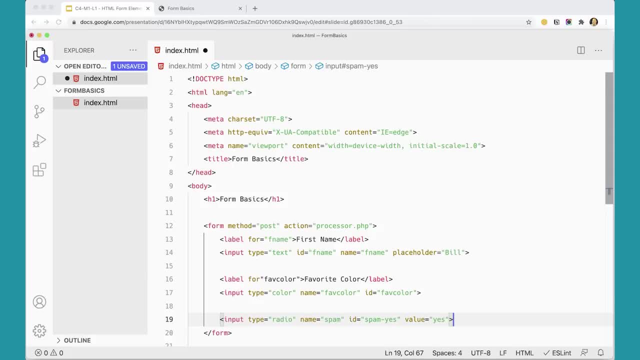 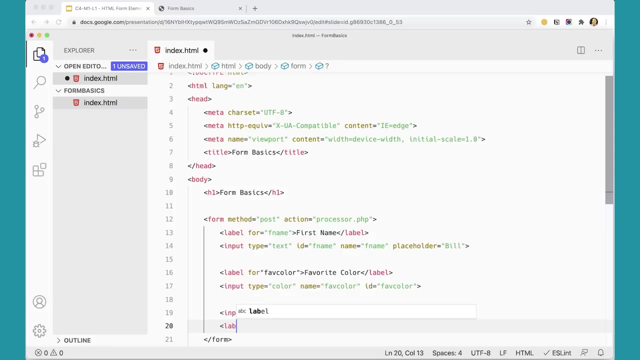 Because When they get sent to the server, you need to know which group it is. You need to know which, what the value of the particular input that was checked is, So that value needs to be set there. And then I'm going to add a label. 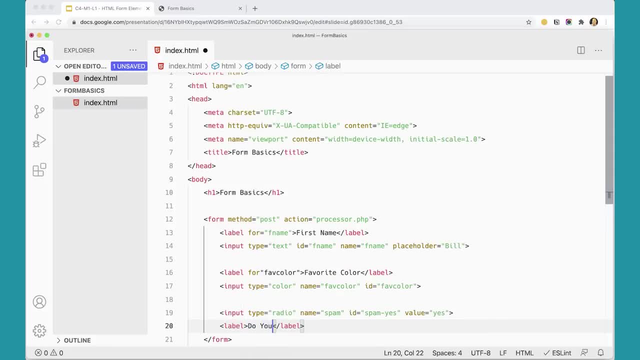 Do you want spam? Yes, We all love extra email, And the label again is going to connect to the ID for spam. yes, So that's one. I'm going to copy it and just paste it to make the next one. 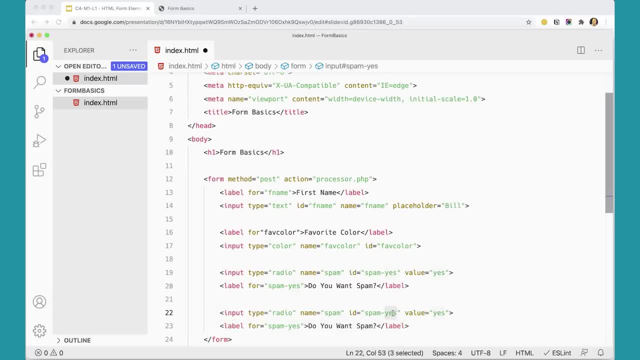 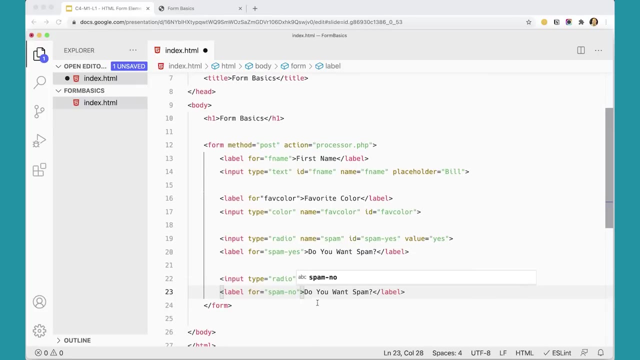 And this one's going to be spam. no, The value is going to be no And this one down here is going to be no. Do you want spam? Yes and no. Or you could put let's say, yes, send me spam. 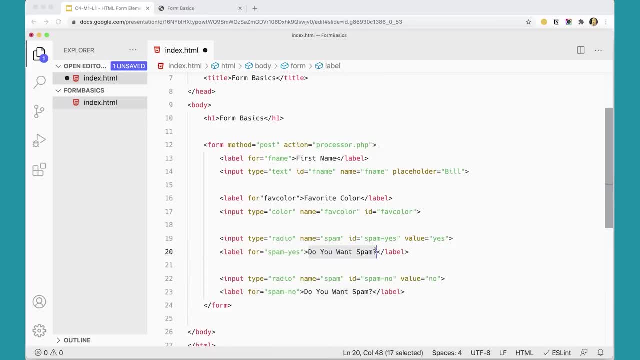 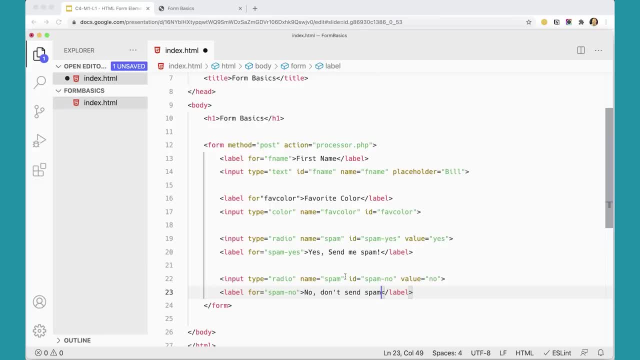 Yes, Yes, And then for this one, perhaps I want this one to be the one that's checked by default. I can put checked and then let's give this a try. Coming back to my form, here you can see I've got two radio buttons, because they are a set. 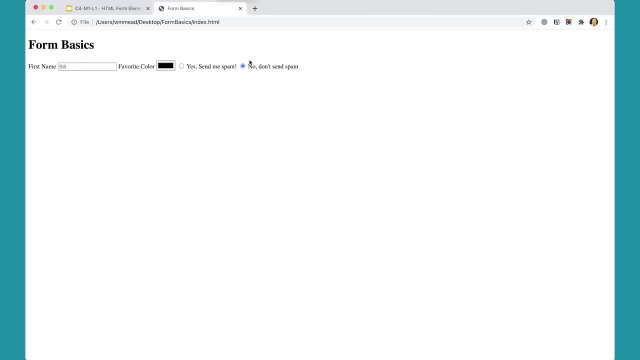 they both have the same name. You can only check one of the two, So I'm going to access it. Then I'm going to move the name Right back over, check one of the two, But this one comes up checked by default. One quick final. 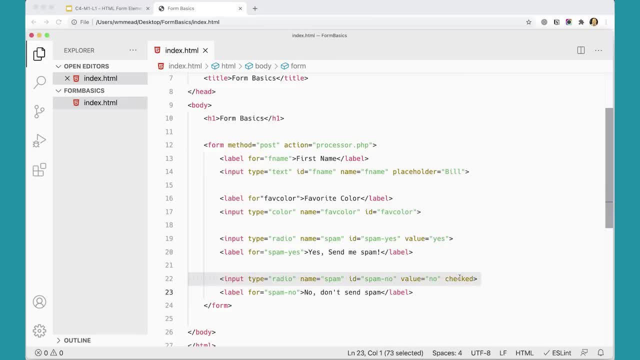 thing about this attribute checked. This is a shortcut for checked equals, quote checked. Probably you learned at some point that whenever you have an attribute in HTML, it has the name of the attribute, an equal sign, and then the value inside quotes. So we have the same thing here. We have the name of the. 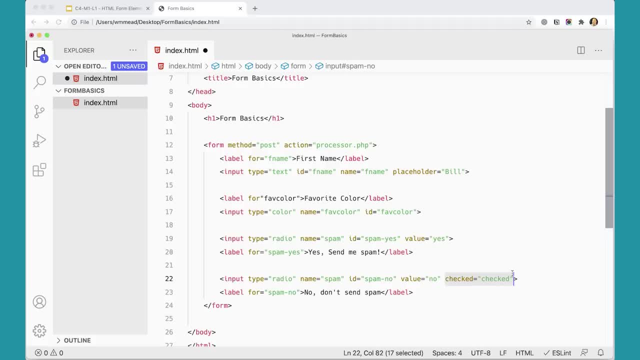 attribute an equal sign and then the value inside quotes. But when they worked on the HTML5 specification they decided that checked equals quote. checked is awfully redundant. So when the name is the same as the value, you can omit the equal sign and the the quoted value in there and just do checked And it's. 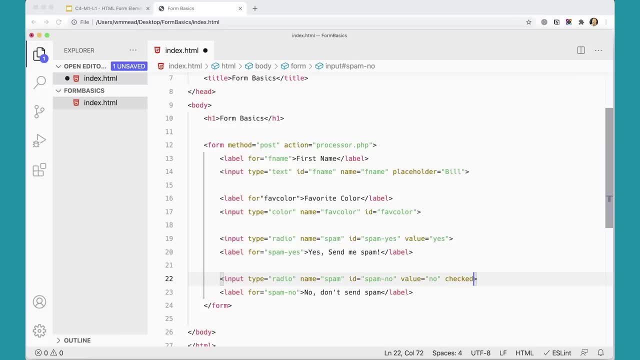 pretty much exclusively in forms. There are a few other places in forms where we'll see this happen, But it's pretty rare that you don't see a name of an attribute, an equal sign and then the value of the attribute. This is just an exception here, because it looks 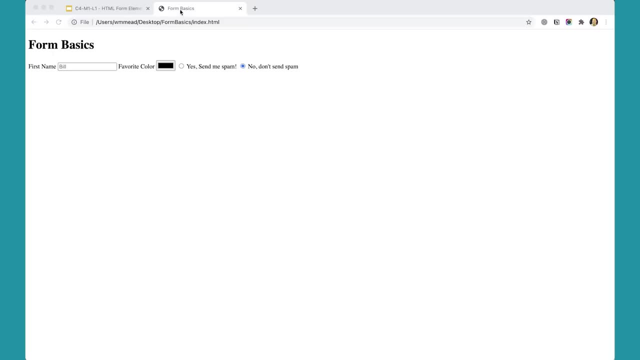 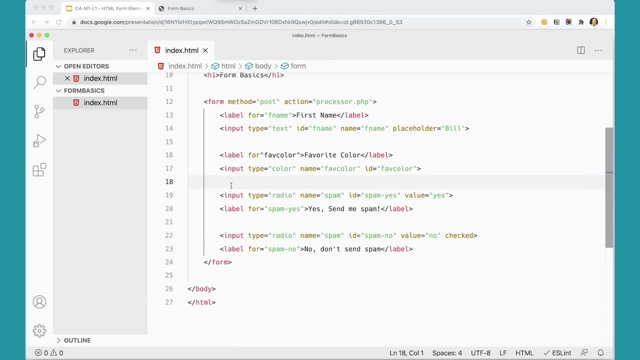 it seems awfully redundant And we want to cut down on those types of redundancies. But you can see that that works just as fine. just fine, Okay, great. The next thing I want to do is group field sets together So you can actually. 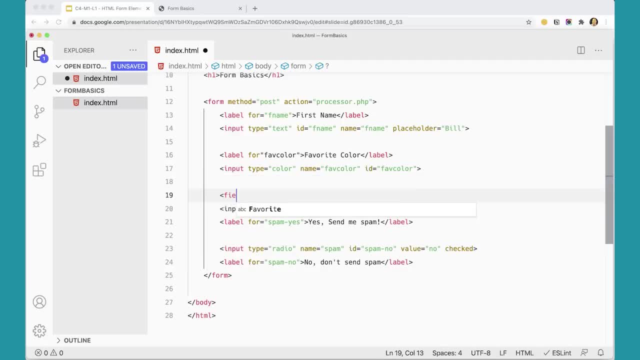 say: alright, this is a field set here, Field set, So I'm gonna, I'm gonna group them together like so, And then you can also add a legend. do you want spam? Yes, send me spam. No, don't send me spam, So I can save that and come back here. 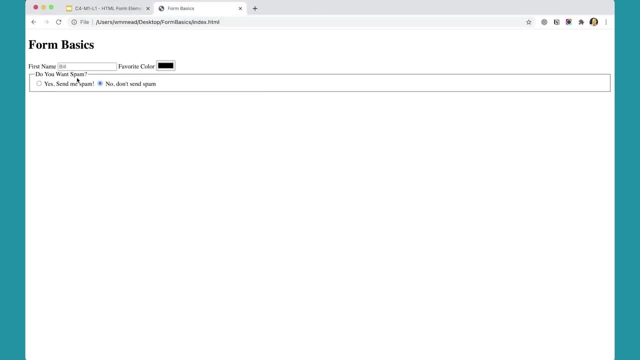 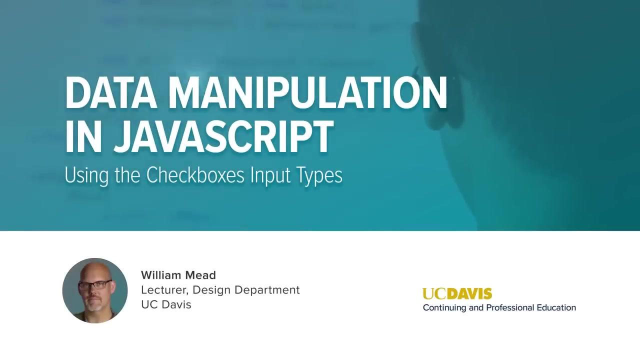 and test it And you'll see. now I have a field set. The field set can be styled with CSS. the same way any other element can be styled By default. it puts this square boxer in here, but you can get rid of that and style it any way you like. Next we'll take a look at how to work. 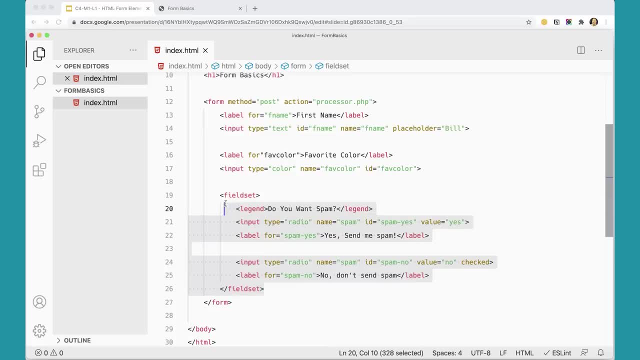 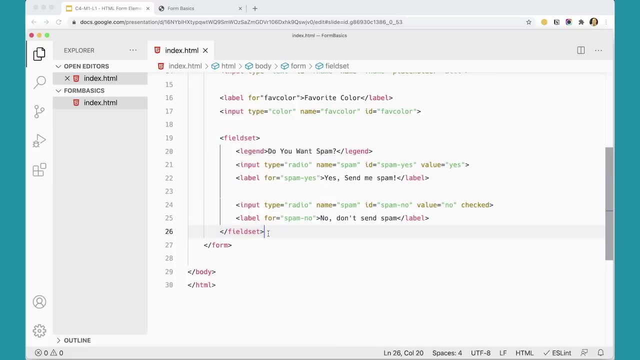 with checkboxes. Checkboxes are different from radio buttons in that you can check any number of buttons. You can check any number of buttons. You can check any number of buttons. So, unlike radio buttons where you can only check one in the set, checkboxes you can check. 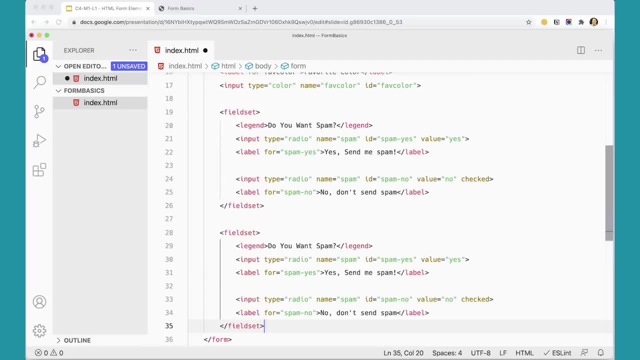 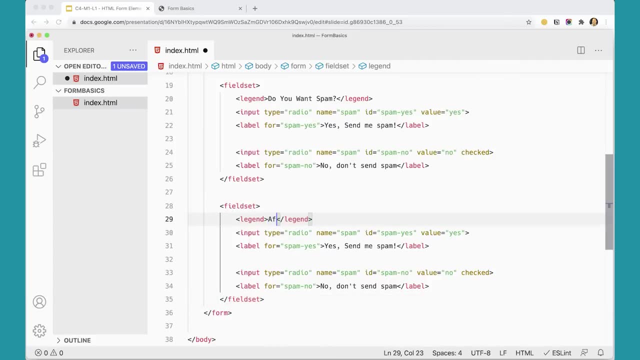 as many of them as you want to. So I'm just going to copy and paste this And I'm going to change this to change the legend to something like favorite animal. I'm having a hard time with spelling today And instead of radio, I'm going to change this to checkbox. 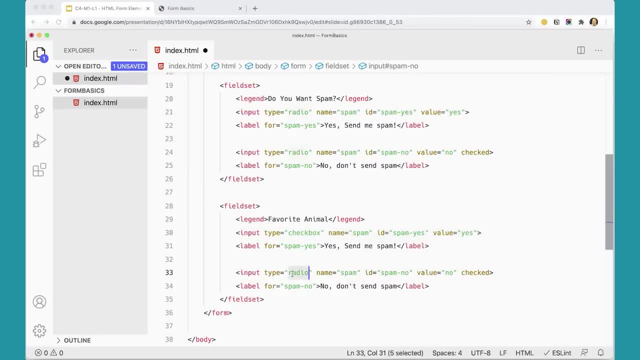 Checkbox And we could give this, you know, a name, cat ID, cat value, maybe cat with a capital C, And then label for cat, And then the value for cat, And then the value for cat, And then the. 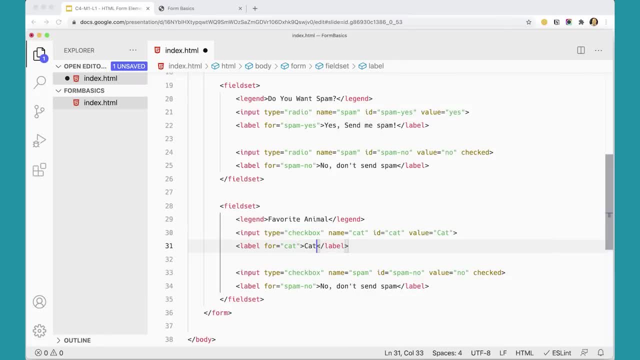 value for the label is going to be cat. So it seems awfully redundant in that we're using cat, cat, cat, cat and cat five times here for this one checkbox. But I could use. I'm going to do the same thing down here. I'm going to. we'll change this one to name dog. 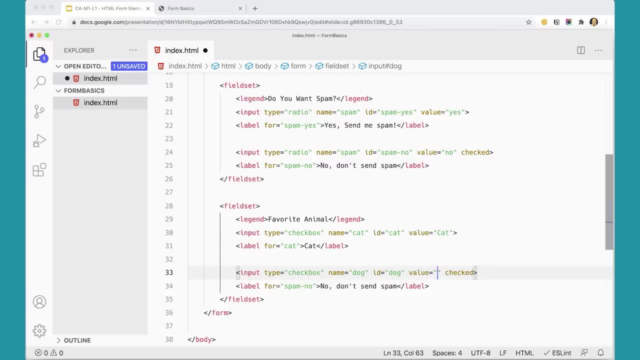 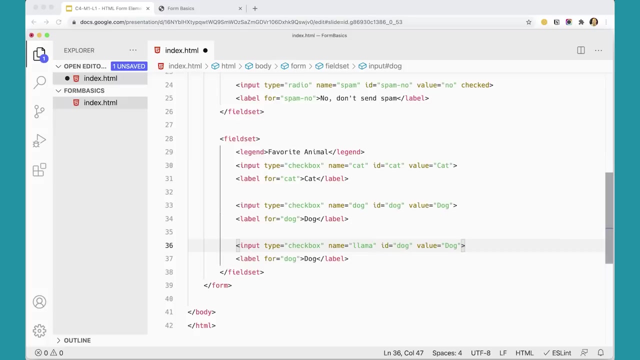 Dog Value. dog with a capital D maybe Get rid of, checked for the moment. Name for dog And then the value is dog. And just for fun I'm going to add just one more: The llama ID, llama value, llama for llama and llama. 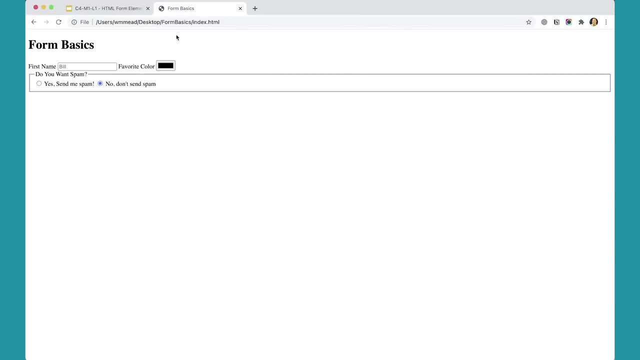 If we come back and test this, you'll see. I get checkboxes and I can check as many of them as I want And that can. that's a different interface and a different type of element there, So you can do that. We can also use checked. 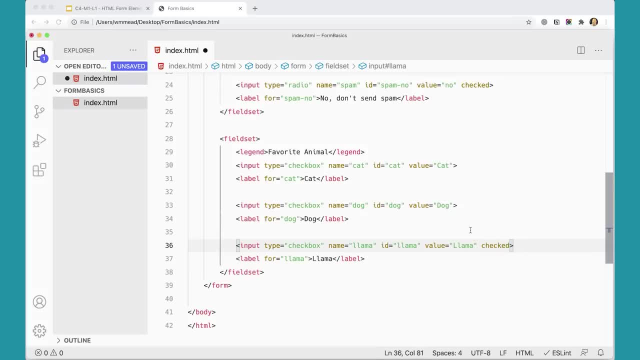 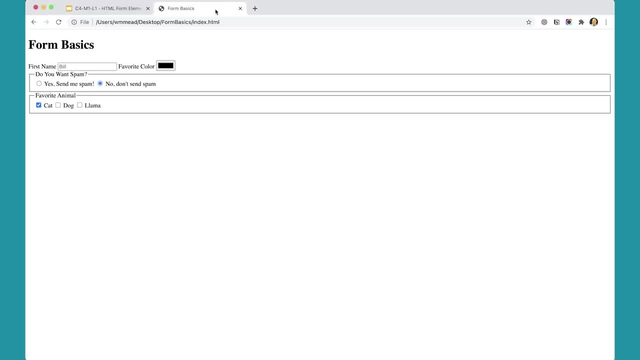 If we want it to be checked by default. So now, if I refresh both of those, it should come back. So now, if I refresh both of those, it should come back. So now, if I refresh both of those, it should come back. 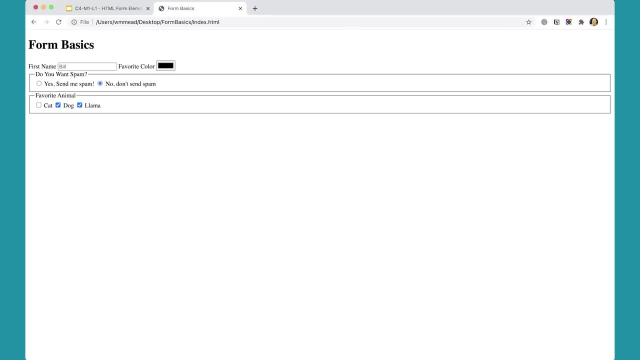 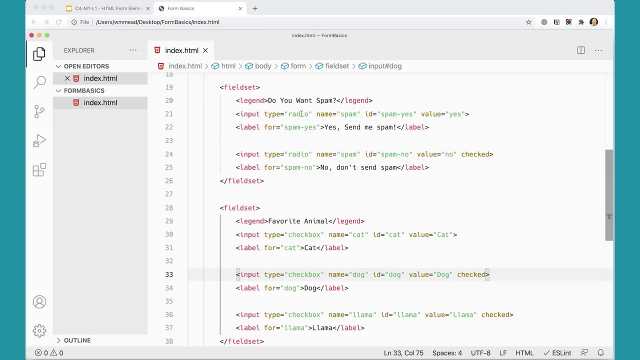 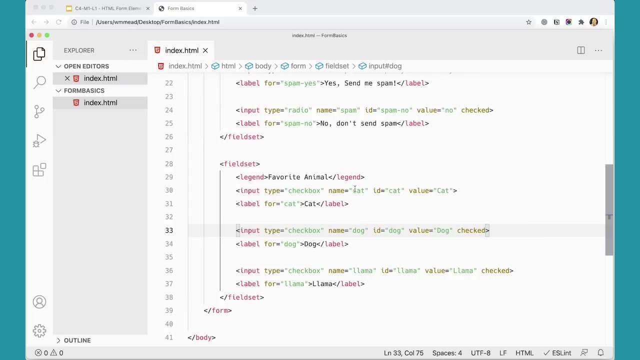 So you can do that. The final thing that's worth mentioning about checkboxes is, unlike the radio buttons that have the name set to the same value- Notice- these names are set to different values. If you want these to be treated in the PHP backend as an array, you can do it like this: 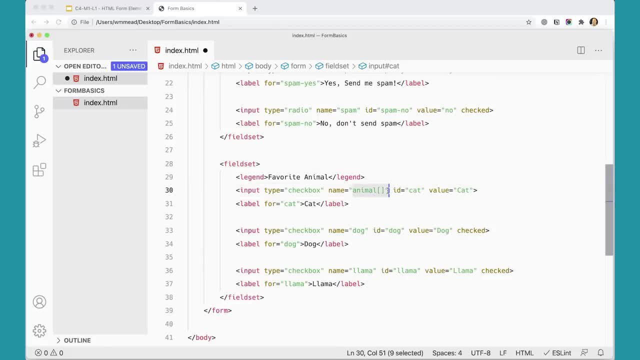 Square brackets. If I name them all animal with square brackets, then it will be treated on the back end when PHP gets the file as an array that you can loop through and work with as a group of items. Sometimes that's useful on the back end and that's one way it works with PHP. 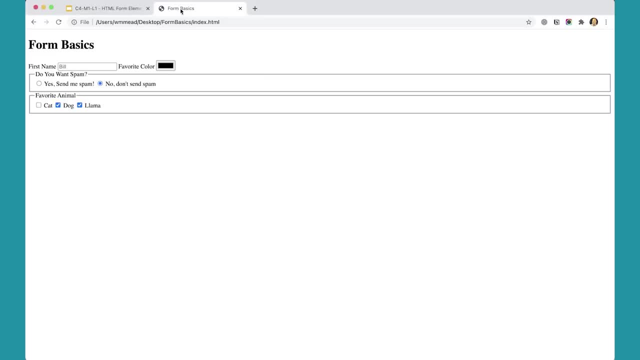 I'm not sure about other languages that will process forms, but in PHP you can do that, And so these are now. would be sent through to the processorphp as an array of items, some of which may be checked and some of which may not be sent as values in that array. 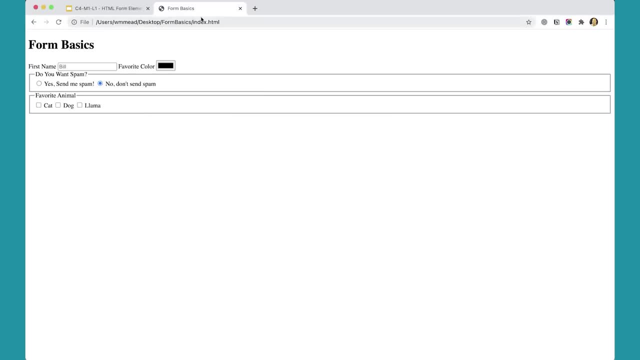 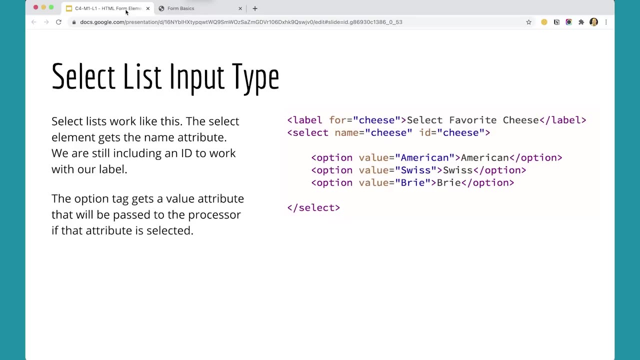 But you can do it that way in PHP. Let's look quickly at select lists, which is another Way of collecting data and can be very useful in forms. So here in select lists we can have a label and then the select gets the name and the ID, and then we can have options and we can set values for these options within the select list. 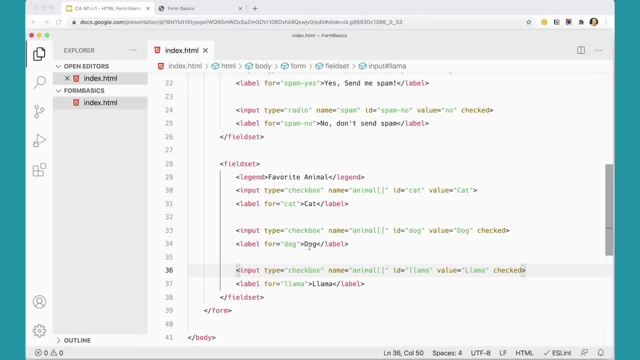 So type one of these out to see what this feels like. So down here I'm going to make after my field set. here I'm going to make the label Favorite cheese and then I'm going to give the label and a for attribute for cheeses. 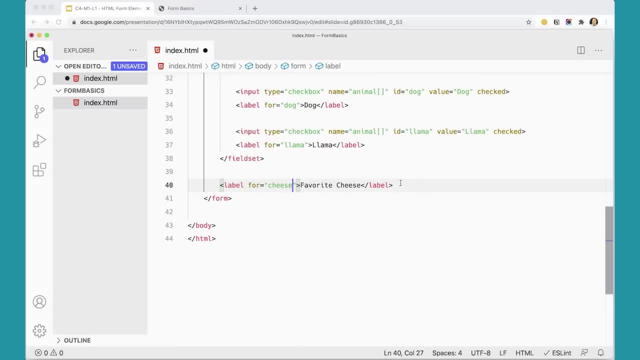 Maybe I'll just do cheese, so you can only pick one. There we go, And then I'm going to set up a select list, select like that, And in here I'm going to give it an ID ID. Oops, ID equals quote cheese. that needs to connect to that for attribute there. 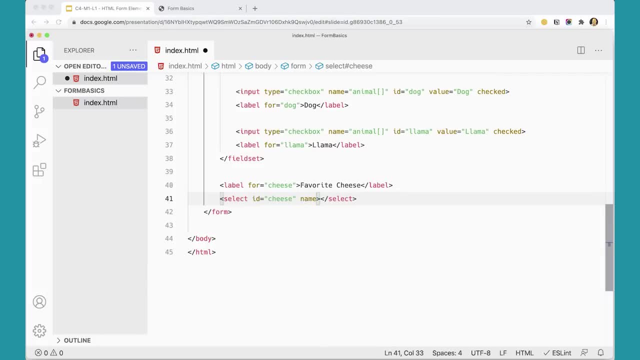 And I'm going to give it a name. Name equals fave cheese or something like that. It could just be cheese And then inside the select list go options And we could say American, And then it gets a value. Each option gets a value. 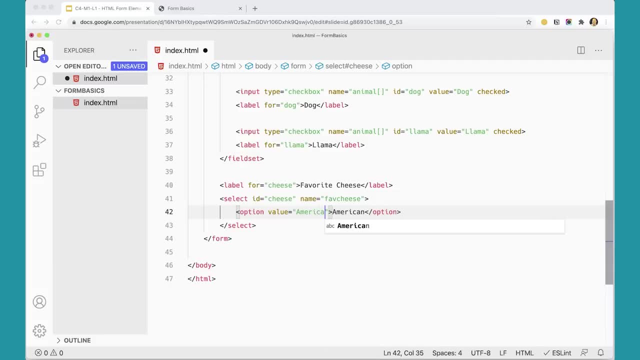 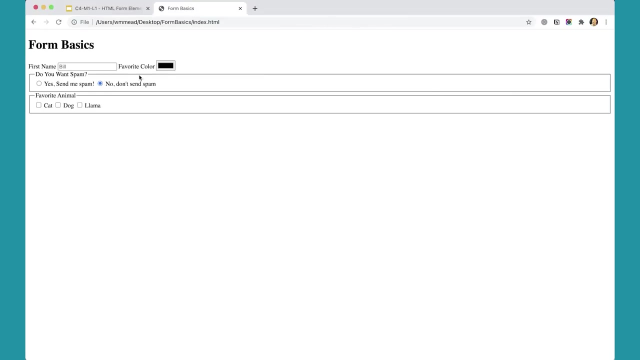 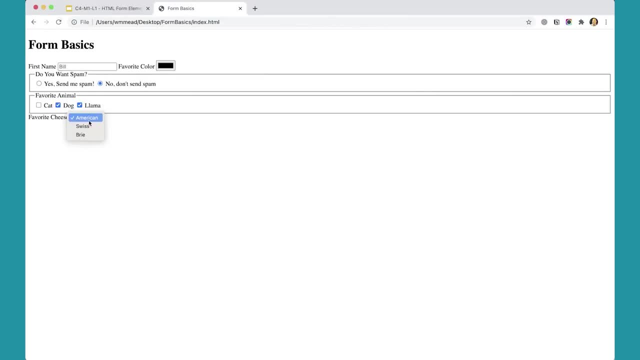 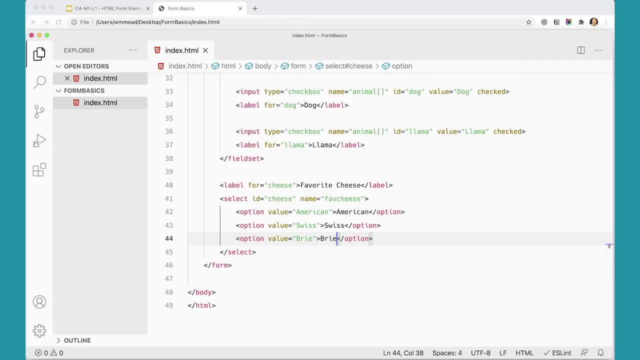 Let's see how this renders over here. Go back over to here and refresh my page. Now I've got favorite cheeses And I can pick from the list. Notice the first one came out checked, selected. If I come back and refresh that, you'll notice Swiss comes up selected. It's the middle. 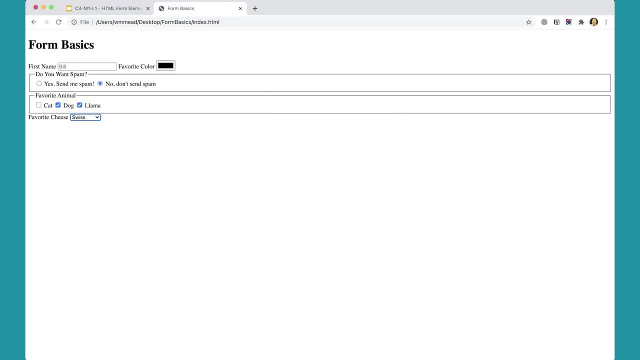 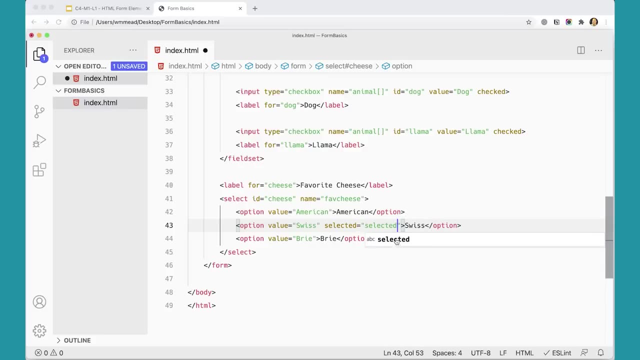 one in the list And again selected is a shortcut for selected equals quote selected. We don't need to type out the whole long thing, We can just use the shortcut selected. It's not uncommon to have the first option, not have a value. 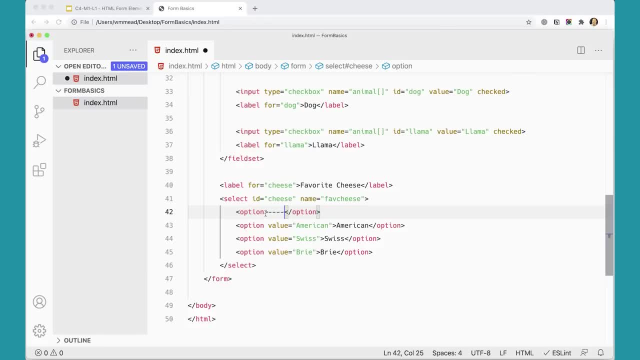 Something like that. So there's no value here And you want to make sure that users pick a value, to make sure that one of these is selected, But you want to start off with no value at the top, So that would give us something like that. 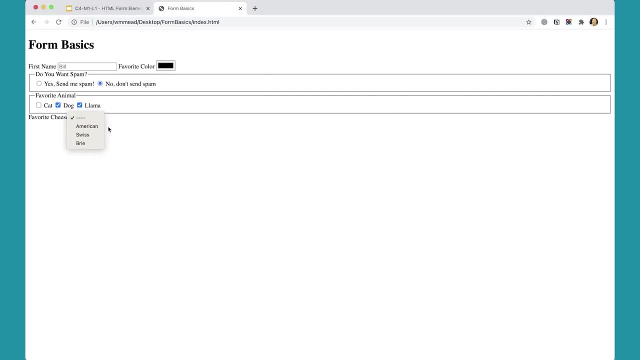 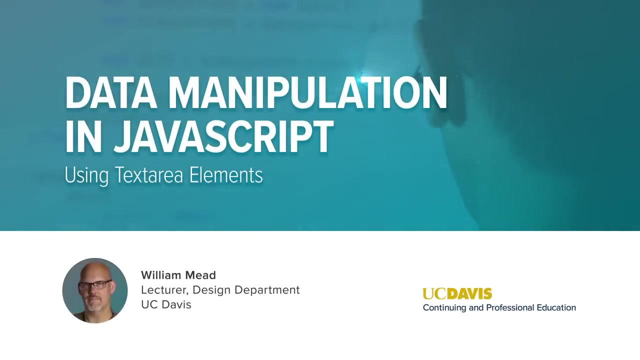 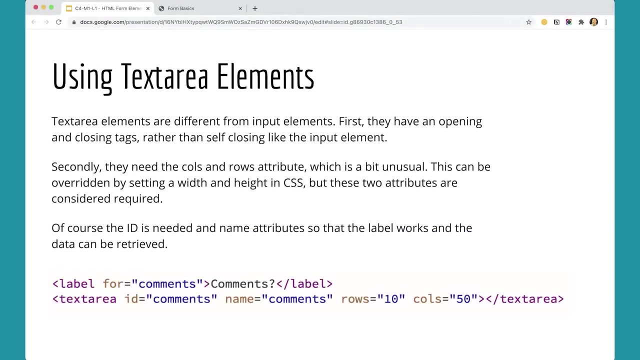 Something like this: And then we can pick one of these And in our form validation we can make sure that it isn't sent through without any value at all. Next we'll look at using text area elements. So let's take a look at this. Text area elements are: 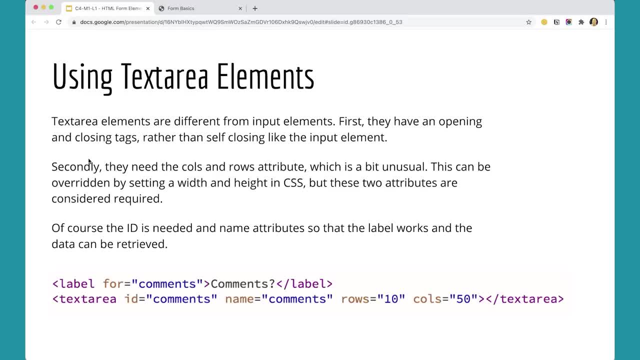 a little bit different from input elements. First, they have an open and close tag, whereas the input elements are self-closing. Secondly, you need this rows and calls attributes here, which seems a little strange because it affects the way the field is rendered in the. 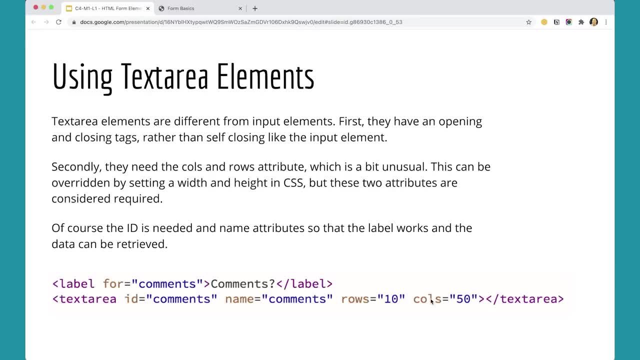 browser. Usually that stuff is done in CSS, But you can override that in CSS. Of course, the ID is needed and the name attribute so that the label works and the data can be retrieved, So we need those as well. So let's go ahead and add this to our 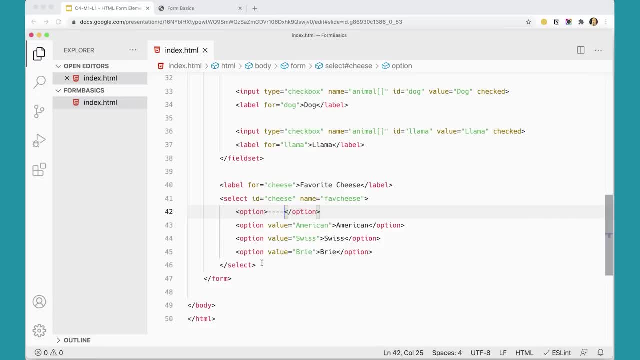 form that we're working on over here. After my select list, I'm just going to add text area, Open and close text area, And then I'm going to add a name Comment and ID, Oops Equals comment, and then a, and then rows equals. maybe 10 rows is plenty, which in quotes. 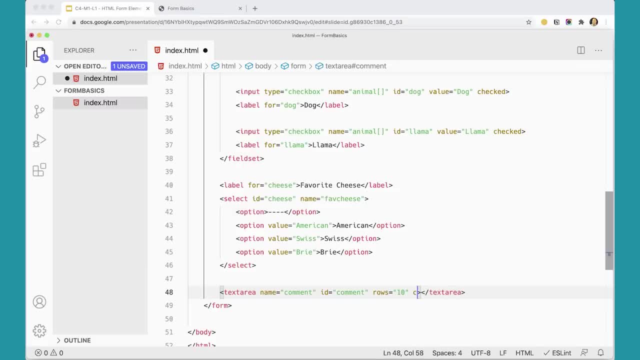 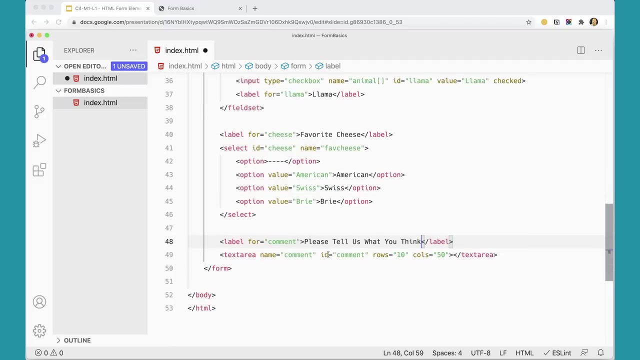 and then calls equals- oops, calls equals- quote maybe 50 columns and that. so that will create a text area. of course we need a label for it, so i'm going to add: for equals comment: please tell us what you think. something like that. there we go, and that will give us a basic text field that we can type into. 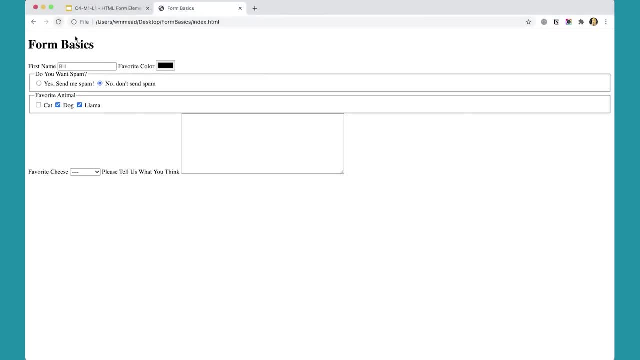 let's check it out. so now i've got, please tell us what you think. notice: all of these are the same text fields that we can type into. notice: all of these are the same text fields that we can type into. these are in line, which looks kind of terrible, but i can type in here: 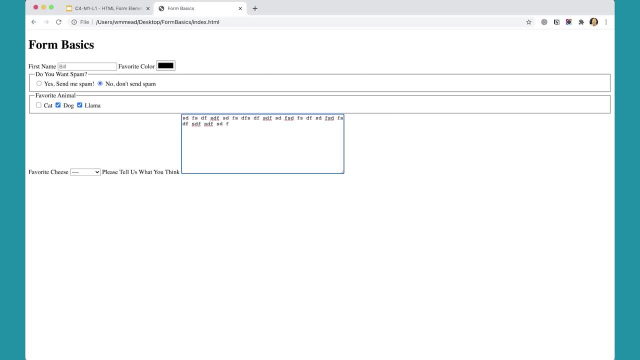 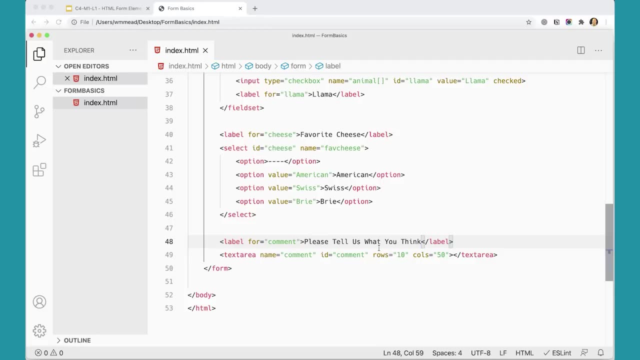 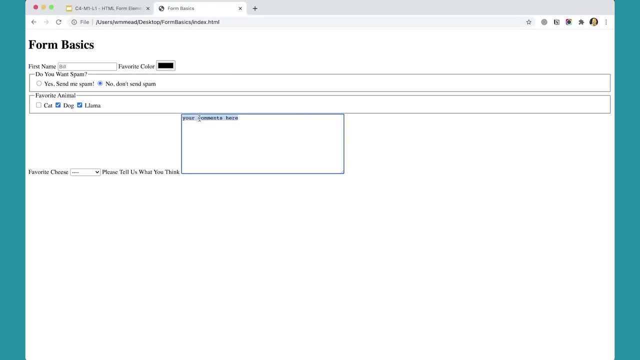 and that will work out just fine. if i want some default text in my field, i can put something between the two text area tags. so instead of adding a value attribute, you would put something in here. so that's another thing. that's different. your comments here now that's actual content that you could come in and change. 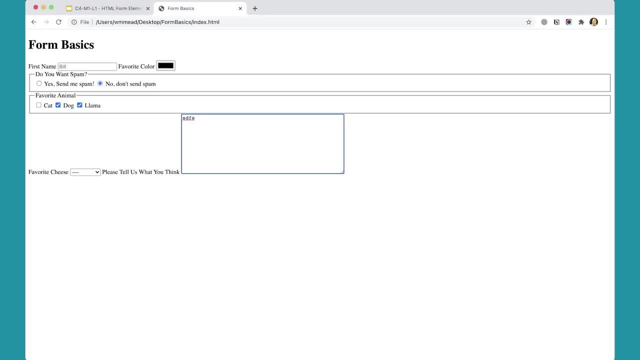 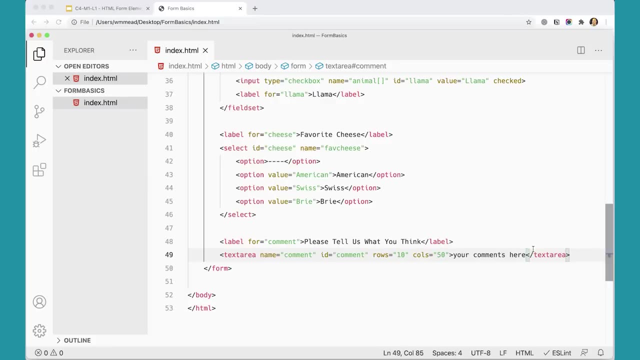 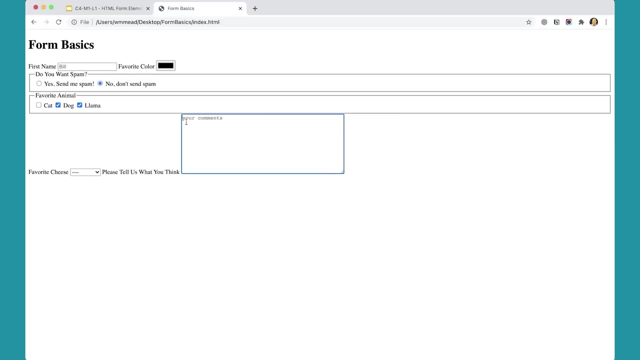 that's different than a placeholder. so don't forget, placeholders are are better for placeholder text. if i wanted to put your comments here, that might be better to put inside of a placeholder attribute, something like that: now when i click here, i can just start typing and that'll go away. i don't have to select it. it's not. 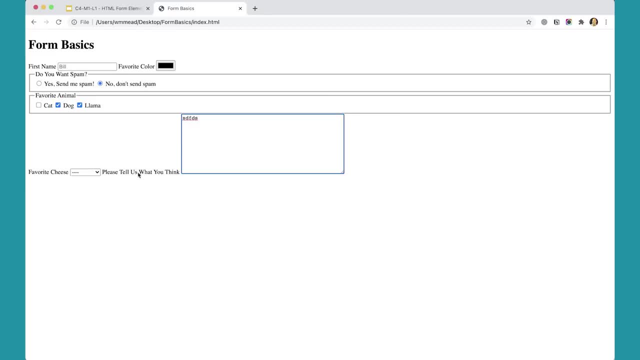 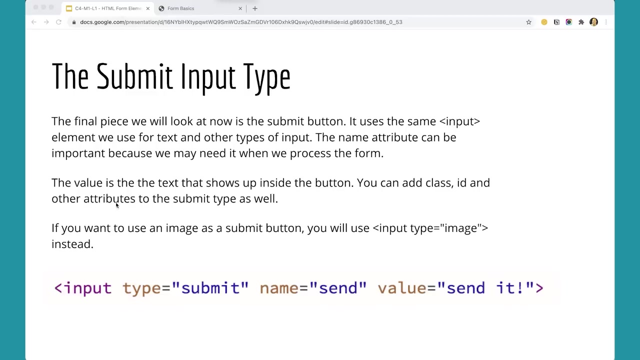 actual content in the field. okay, great. so that gets us a um, a text field. our styling here is pretty awful, but it is functional and working. the last type of field that i'm going to talk about is back to the input type, and that's the type of field that we're going to talk about in this video. 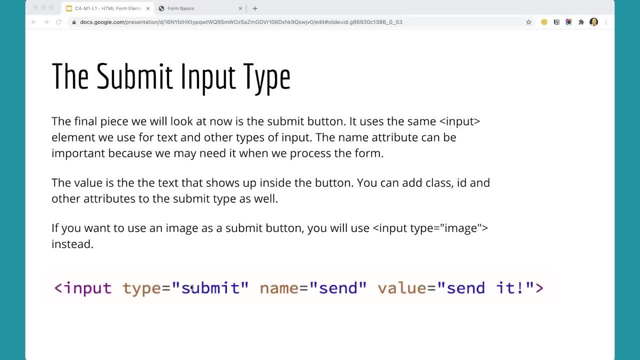 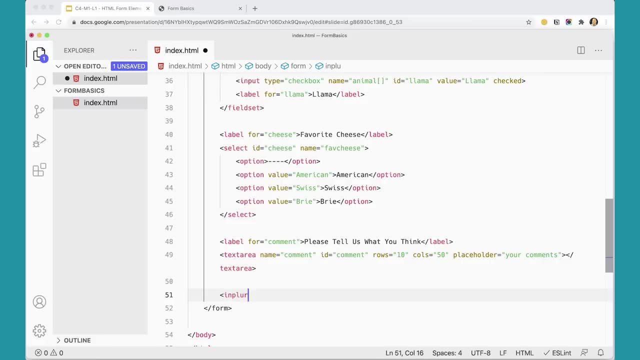 but it's the submit button. this is what actually sends the form to the actual, to the actual form processor. so let's go ahead and add one of these to our file over here. so down here i'm going to add another input, input like that, but this one instead of type, text or color or something like. 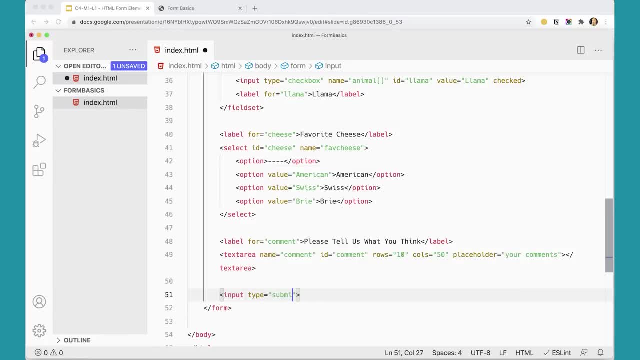 that it's going to get a type: equals- submit, and you can give it a name: name: equals, submit. you could give it an id if you wanted to. id equals, quote, submit. you can give it a value, value- equals send, form, something like that, and you'll notice this will actually create a button on the page. let's go check it out. 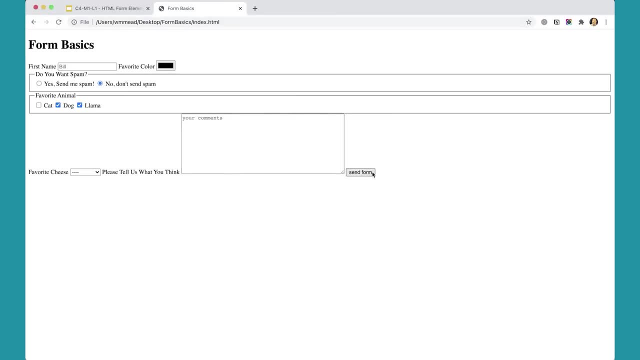 so that creates a button. Notice the value is what gets printed on the actual button send form. And so that will actually take whatever data somebody types in here and send it to the processorphp. Now it says processorphp couldn't be accessed because we don't have a processorphp file in our folder. 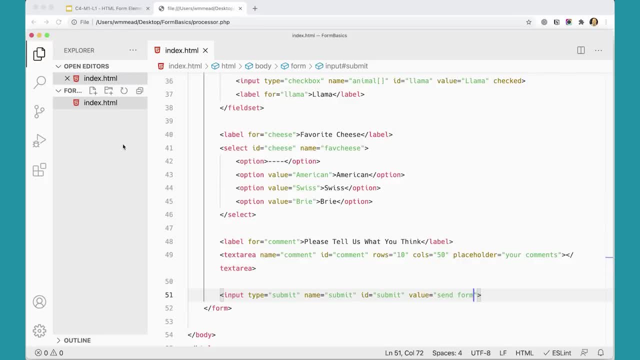 So it's looking for a file here called processorphp, And for PHP to work it has to be on a server, And I'm just working locally on my desktop, So it wouldn't even work if I had one. But if we put this up on a server and the server had a processorphp file here, we could actually capture this data and do something with it. 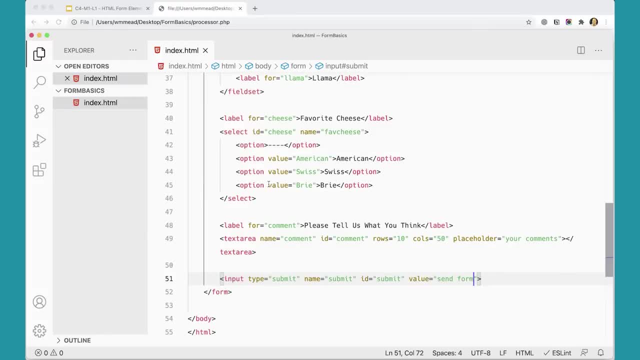 And that would be kind of an important thing to be able to do. Now there are a couple other things you can do. to submit forms, You can also use input type image. So if you want to set an image as As a button instead of the having the browser render a button, 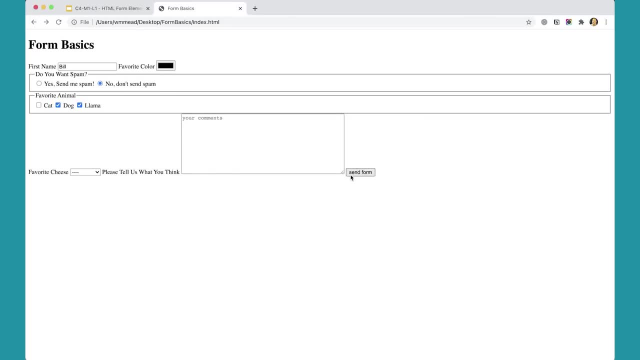 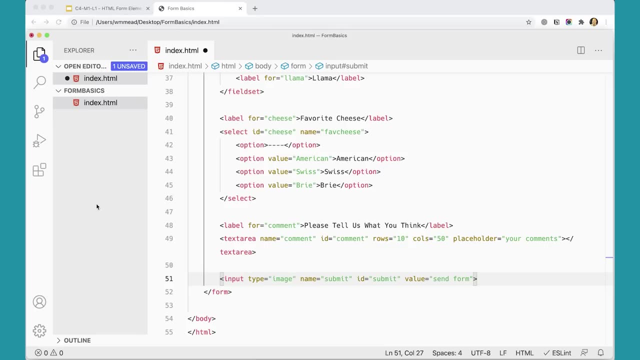 Like this one. you can actually. You can actually use the image there. You can actually use the button element if you want to to submit a form, But the most common way is type submit. It's the most common way And then 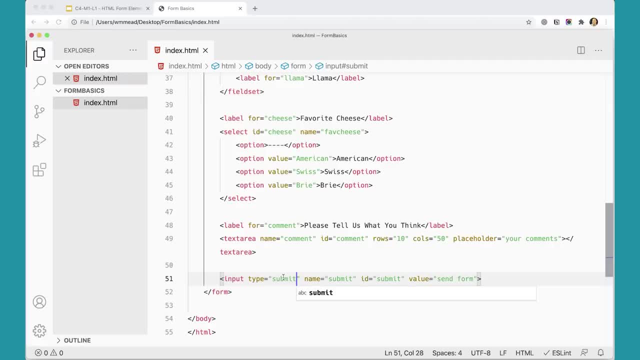 Secondly, you could also add an input type reset if you wanted to put a button on the page that will empty out the form. Generally, it's considered bad practice these days to use reset buttons. I mean, it's not very often that somebody fills out an entire form and then says you know what? I really kind of want to do that again. 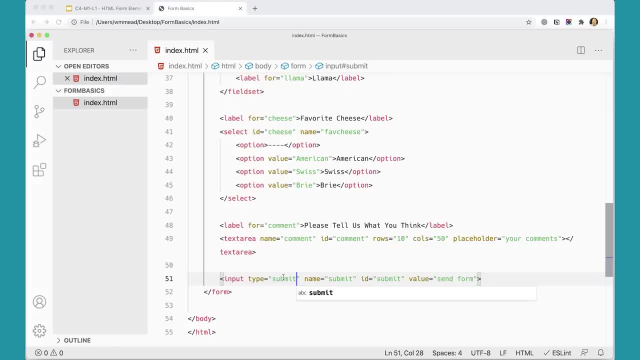 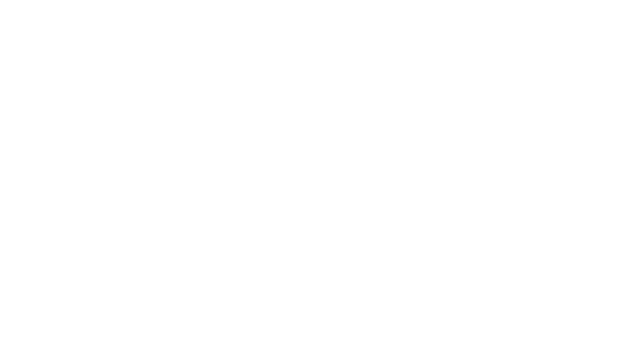 So I'm going to just click reset and fill it out again just for fun. So we don't use reset buttons much these days in the web, but they do exist. So I'm just going to go ahead and turn this one off And then we will. 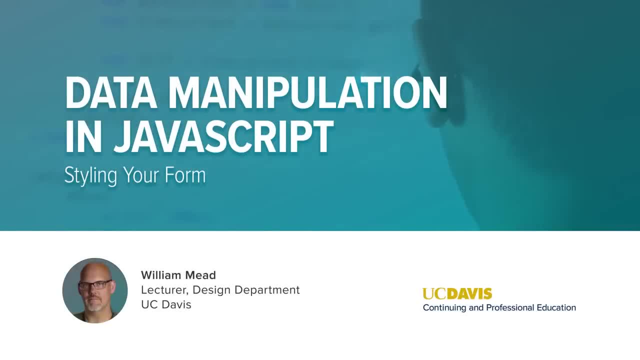 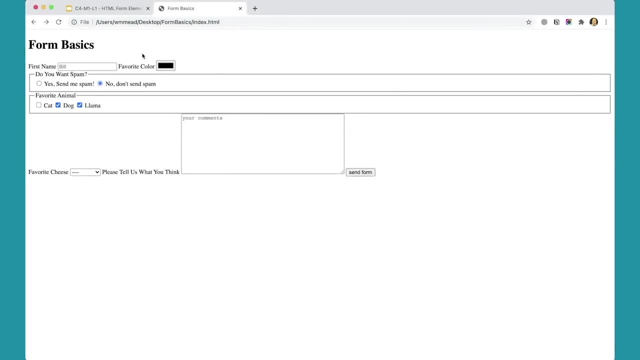 And then we'll go back to the timeline. So once you've got all of the settings ready, then you're now done with your year. at the end of your year We're going to go back and do it. So I'm going to do a little bit of setting here. 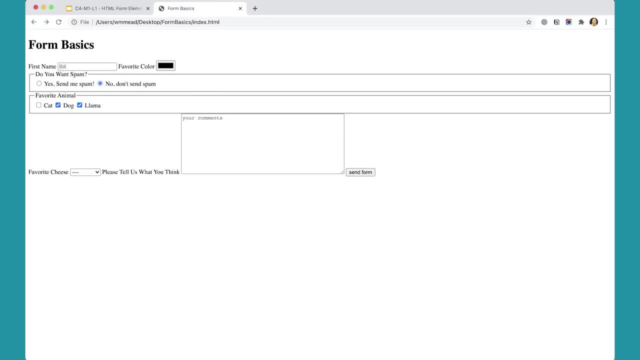 And then you're going to find a little bit of setting that is just perfect to pick out on your page or whatever. So I'm just going to click And then I'm going to go ahead and say I'm really not sure what I'm doing here. 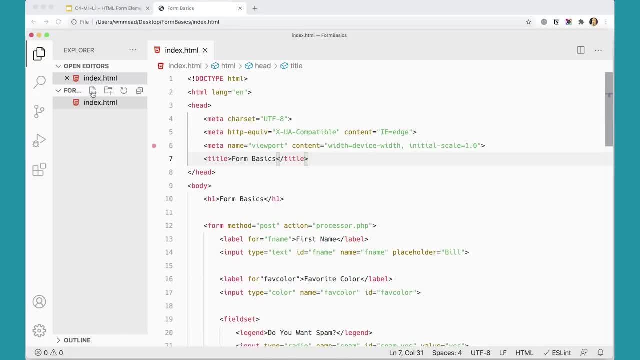 out So I could link an external style sheet here. but I'm just going to add style tags to just do something kind of quick here, And in the style tags I might add something like input comma labels. This will apply to both of these display block And that will help with the 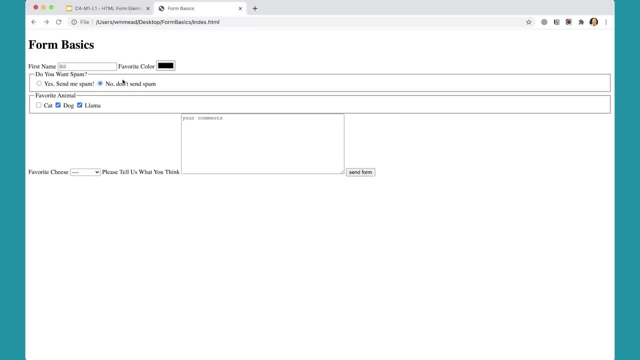 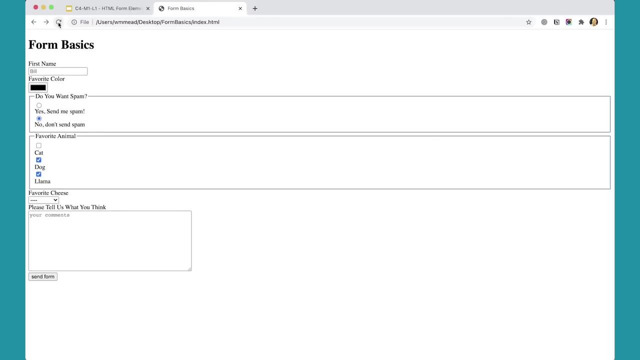 display of the form considerably, because instead of having everything go in line except these field sets, which are block elements by default, that will make all the labels and the input elements turn into block elements like that, And that really helps quite a bit. Now, 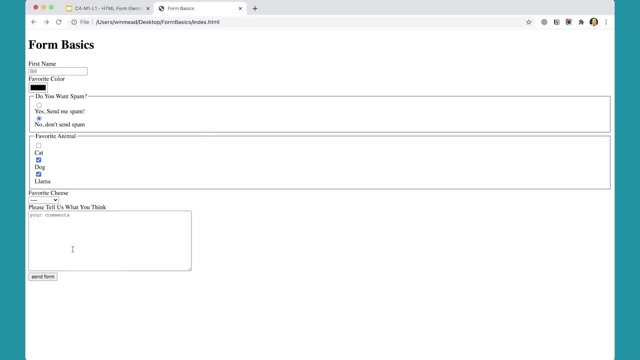 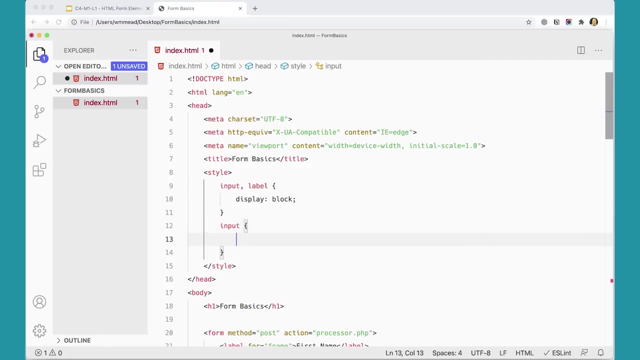 they're all kind of squinched up together. So what we can do from here is add a little bit of margin on the bottom of, maybe, the input elements, So we might do something like this: Input Margin bottom 15px or something like that, And see what that does. Now it's starting to get a. 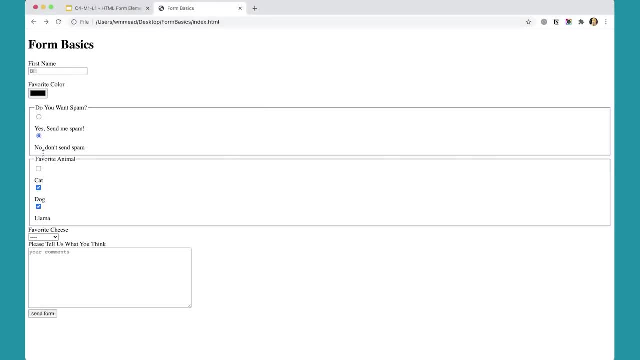 little bit better. This looks kind of funny in here, So we might add something for these field elements. They don't sort of line up this way. Maybe we want to leave those as in line, So I might add something down here for that. 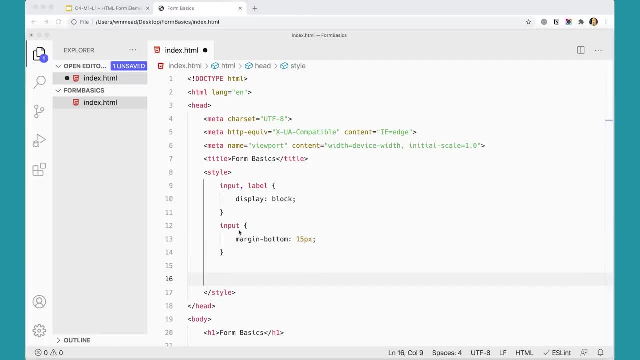 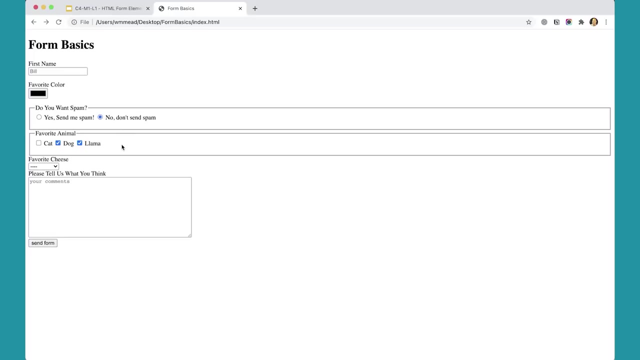 Field set input. Field set label. So if the field is inside of a field set, in this case, I'm going to set them back to display in line so that those look a little bit better. And there we go, Those are lining up much better And we could do a lot again with forms to really help them. 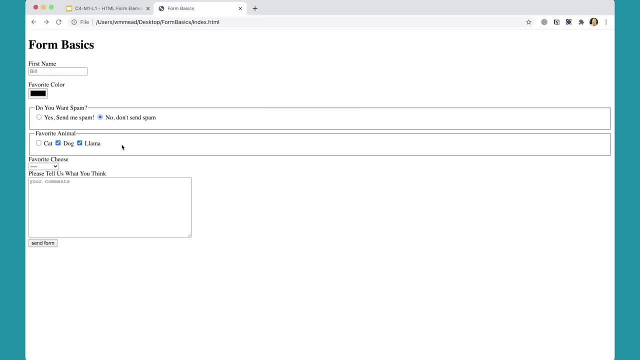 with the display of the form, So we might add something down here. Maybe we want to leave those ways, But theita has so many different ways to improve the way they look. We can- we can do a lot with styling to forms. You could spend a long time getting forms to look the way you want. 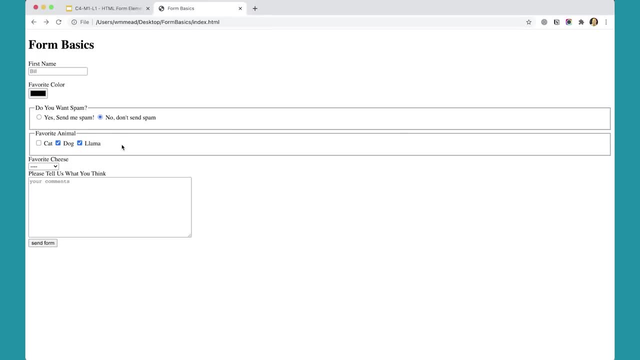 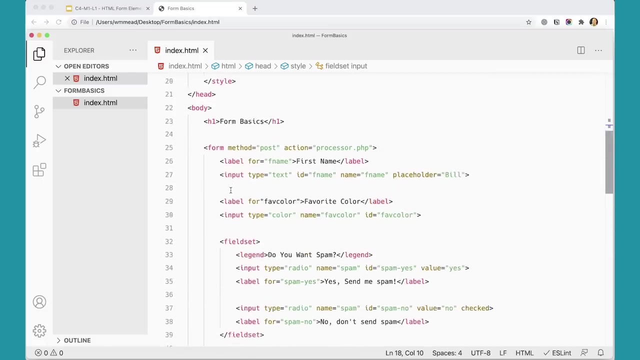 And that's an important thing to be able to do. But even with just a few styles, you can do a lot to improve the overall look of the form, And that's really great. Now, uh, the next thing is, we can also in in our forms, we can require elements. So 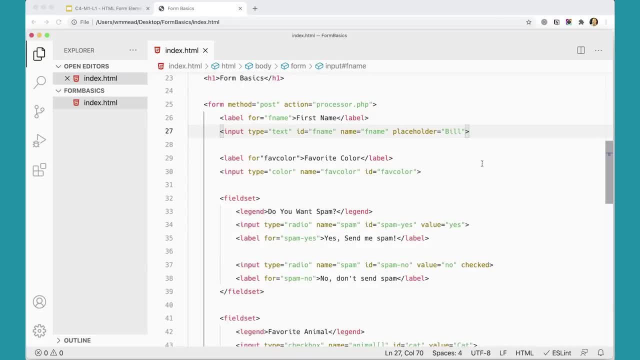 We're going to talk more about form validation in our next lesson, because that's kind of our next important topic. But what I can put in here is I could put something like required, So I have to spell it right: Required, And that again is short for required. equals, quote required. 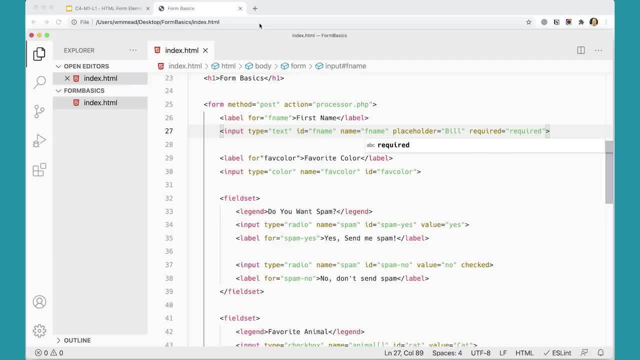 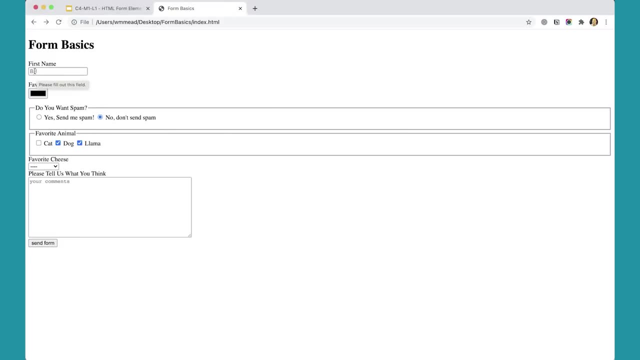 And what that will do is it will make it so that when I try to submit this form, if I don't put something in here- and currently that's just a placeholder text field- if I click send form, it will say: please fill out this field. 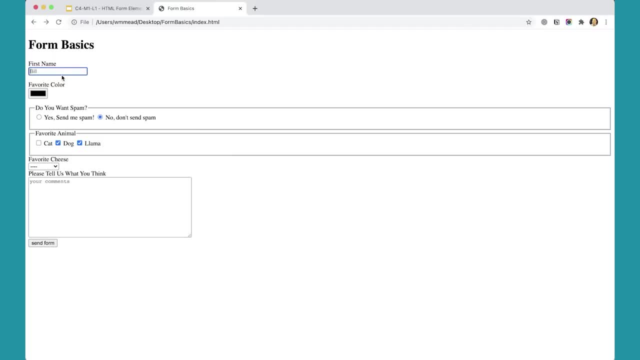 Now this is being provided by the Chrome browser, and different browsers will support this in different ways and put different styling for this kind of thing, But it's important to note that it's not a form that you can put in here. It's there. 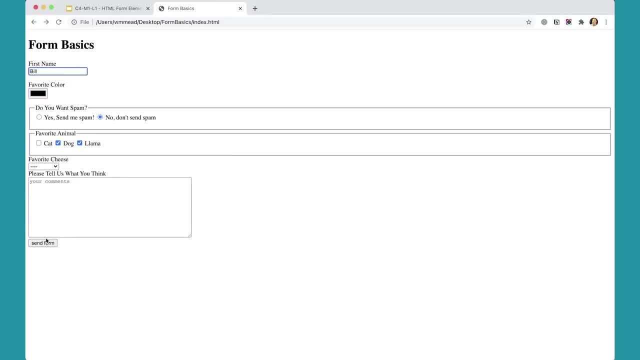 Of course I don't have an actual form processor. So if I do fill out that field it's going to try to send it and it doesn't have anywhere to go. But it won't even try to send it if I don't have the field filled out. 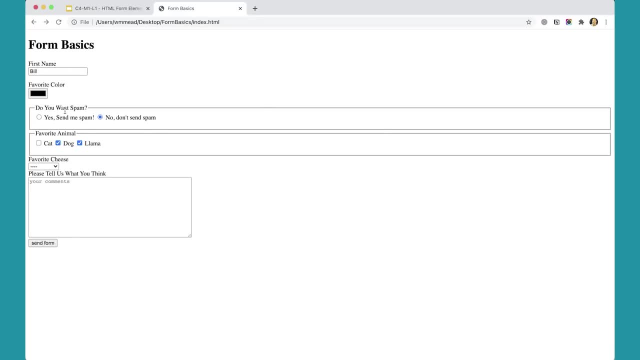 And that has to do with form validation. Form validation is the next thing that we're going to look at and is a very important part of collecting data from users, because we want to make sure we're collecting the correct data from users. We want to make sure that we're collecting the correct data from users. 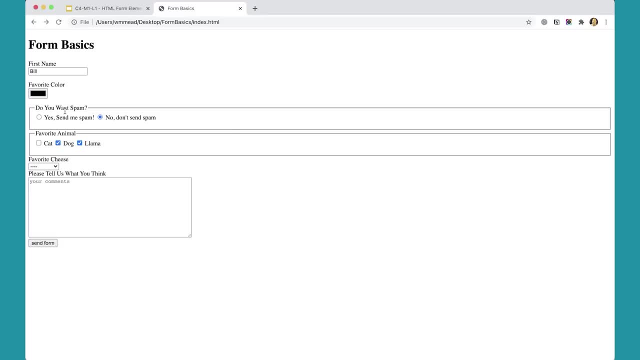 We want to make sure for ourselves and that we're protecting our back end from bad data, And we want to make sure for our users so that they're filling out the forms properly and they're having a good user experience on the front end as well. 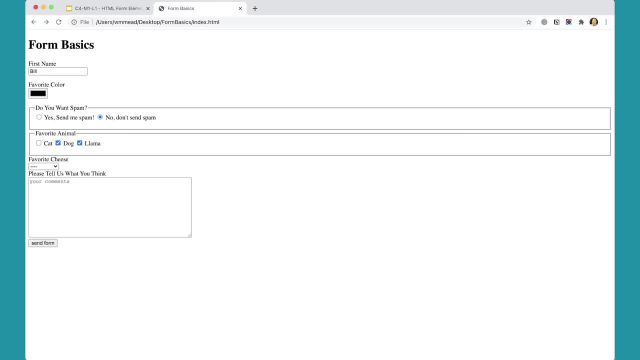 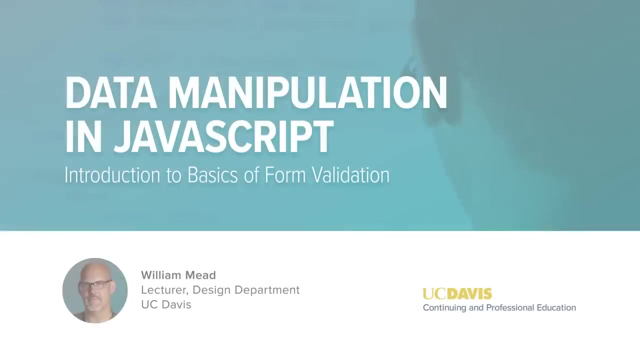 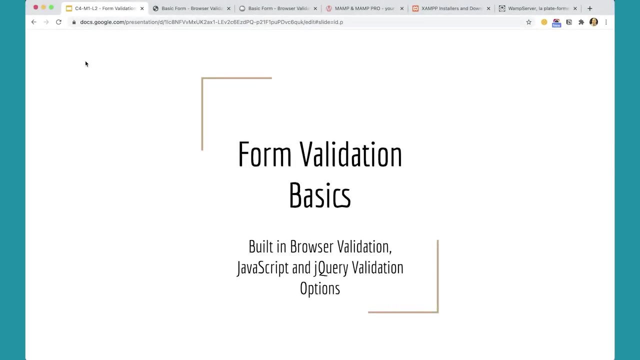 And that gives you kind of a quick overview of how forms work in HTML And they're very useful and we'll be using them a lot on any kind of website or website web application. Form validation basics built in: browser validation, JavaScript and jQuery validation options. 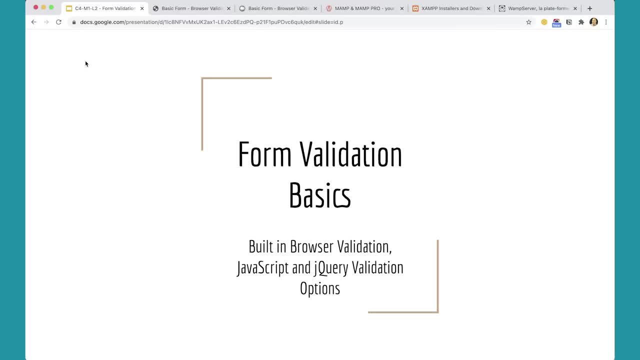 In this lesson, we're going to take a look at how we can validate forms, And form validation is one of these things that's maybe not the funnest thing in the world or the the fanciest thing in the world, but it's really. 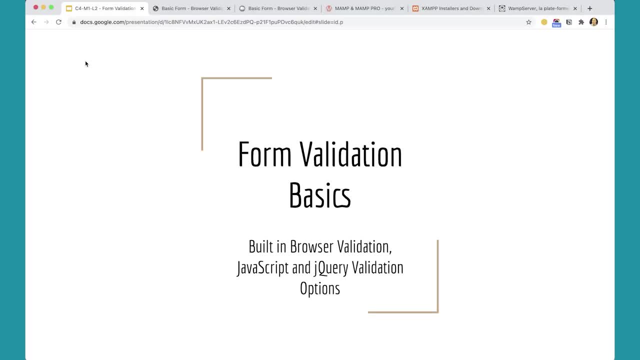 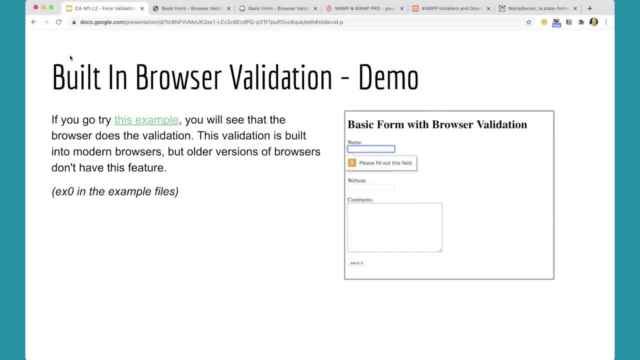 really useful And it's really important that you help users by creating forms and validating forms in ways that really help users be able to submit their data, because nobody likes to fill out forms. Nobody wants to spend their time doing that. First of all, there's in-browser validation. 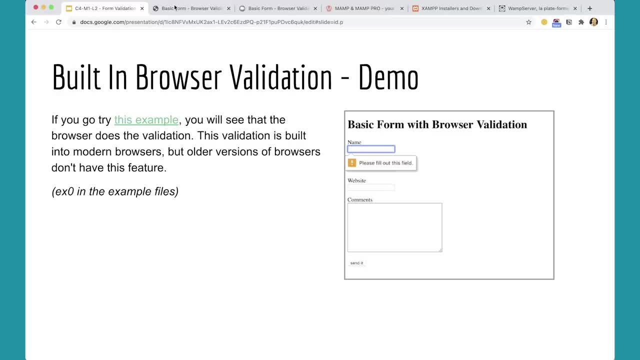 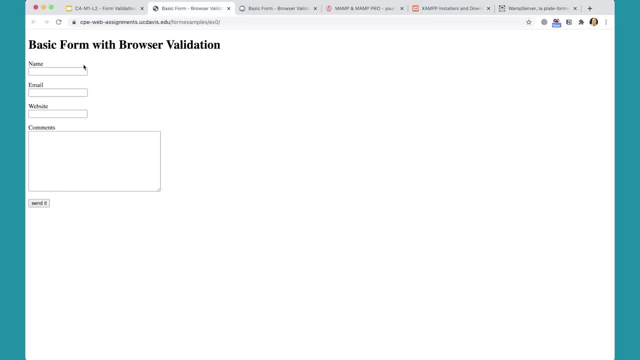 And I have a demo here and this example is here And I will give you these links in the lesson so you can check out these examples here. But if we click in here and or if I just try to send this form with no information in here, 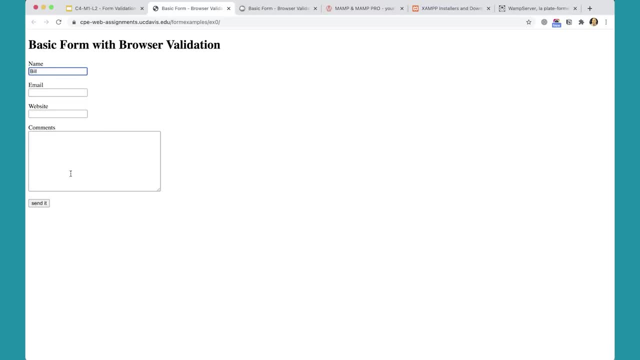 it's going to tell me to fill out my name. If I fill out my name and click send it, it's going to tell me: please fill out this field. If I put something in here other than an email address, it's going to say: please include an app in the email address. 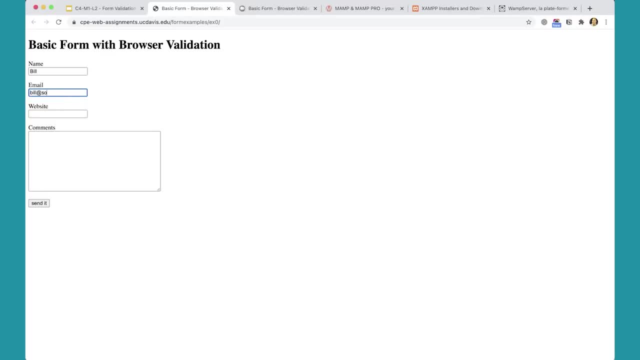 So we want to do you know bill at somewhere, dot com, something like that. If I click send it it's going to tell me I need to fill out a comment. The website is optional, So if I click send it, you'll see it goes through. 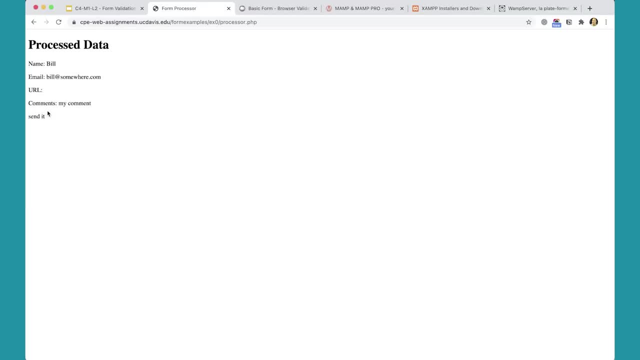 The URL was optional so it didn't require it, But but it did go through and I'm getting this processed data and this is being processed by a PHP file on the back end. And this is only front end validation. We also need to do back end validation. 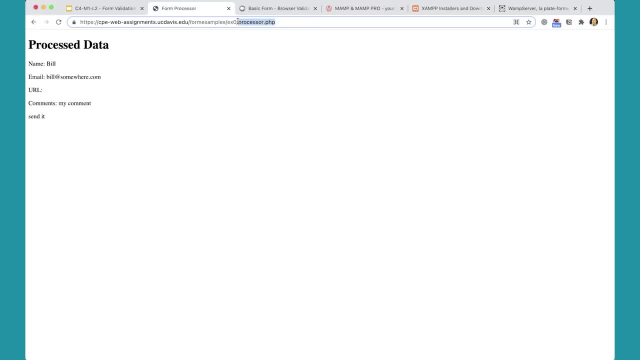 We'll get to that in a minute. Let me go back to the previous screen and show here again: if I put in bill and an email, If I put in a bad URL for a website, it won't let it go through. It's going to say: please provide a URL. 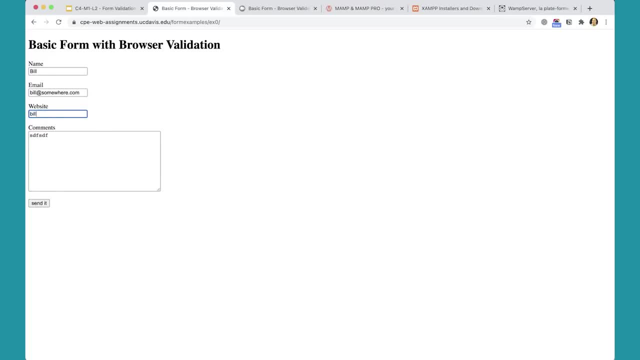 I think it has to be. I can't even just be Bill's site Dot com. I think it needs to have the full HTTP colon slash slash on there for that to actually work. And now, finally, that's going through. So this is just using front end browser validation and 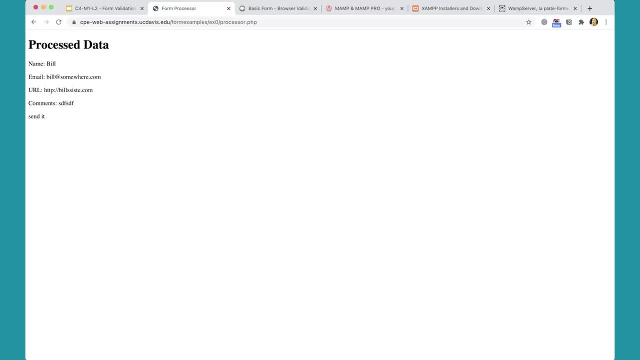 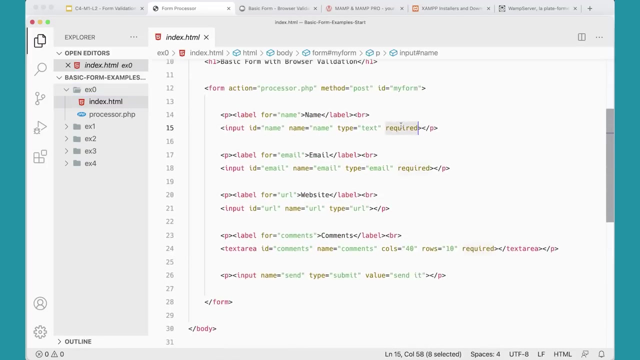 validation provided by the browser. So if we go, look at these files and I'll provide these files for you to check out. If you look in The X zero file here, Make sure you're in the right file here. OK, You can see that I've just set required here. 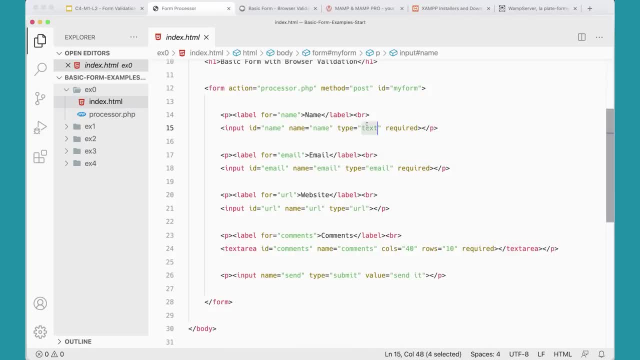 This one is set to an input type text, Whereas this one is set to an input type email. So that's why I did the double validation there and saying that it's it's required, And then if you put something that's not an email address, it says it's got to be an. 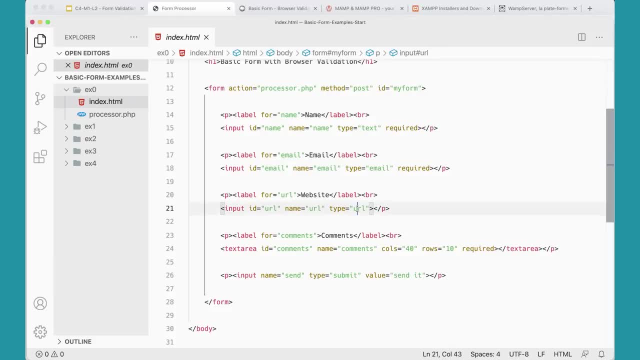 email address down here. This one doesn't have required on it, but because the type is set to URL, it won't let you put a data. put data in that doesn't look like a URL And then the comments are required. So this is just using the built in browser validation. 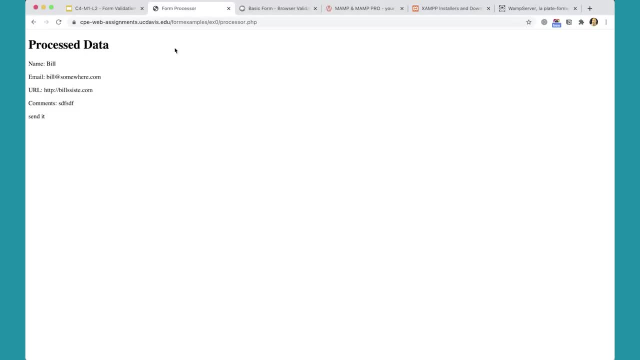 And if you in the process of doing your lessons, if you see something that looks like this type of styling, then it's. it's using the built in browser validation And it looks at this way in Chrome and it might look a little bit differently. 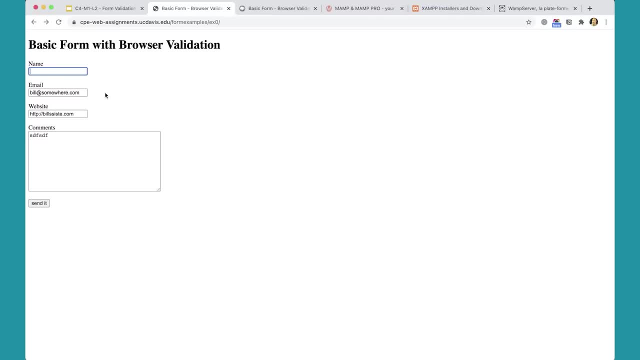 in Firefox or Safari or Edge or some of these other browsers that are out there. There are a lot of other browsers are out there. Those are just some of the most popular ones, or it might not work at all, So that's something to consider in using the built in browser validation. 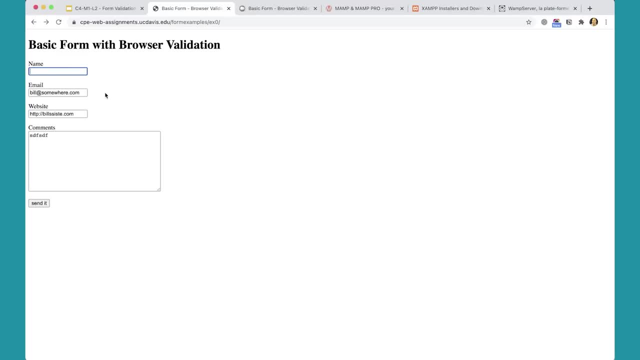 And validation is one of these things that started in JavaScript and has moved into either CSS or HTML- and that's a very typical sort of movement for common technologies in the web world- is that you know to do it, initially you need JavaScript and then and then eventually, some of the features. 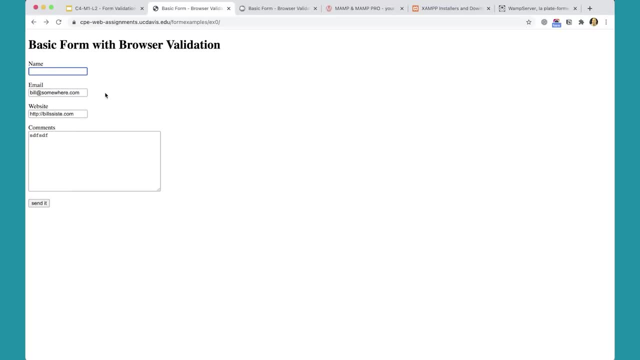 or even maybe in some cases, all of the features end up moving into plain HTML or into CSS, So that's pretty normal, But if we want to take full control over our browser validation, we're definitely going to need JavaScript for that. It's important to note, before we finish up with this video, that required this. 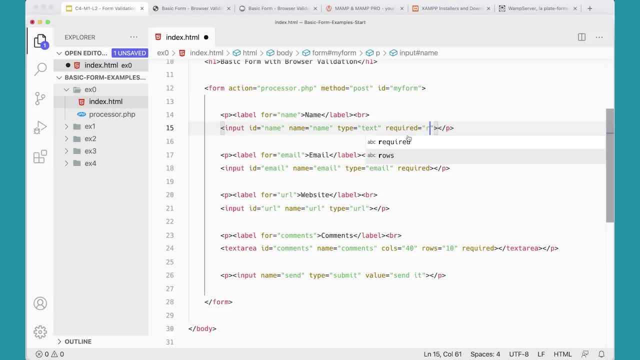 attribute required here is short for required equals quote required. It's a shortcut because in HTML5, they decided that if the name of the attribute is the same as the value, you can have a shortcut. They're just putting required. So that's important to note here. 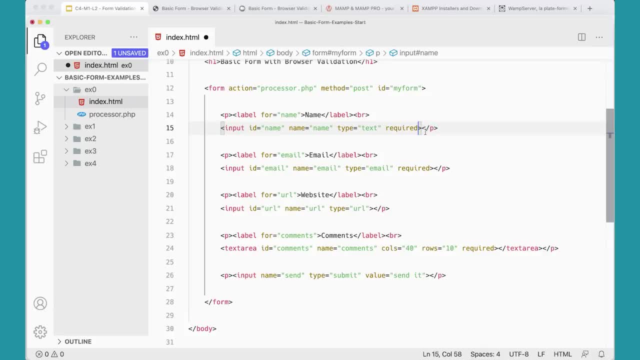 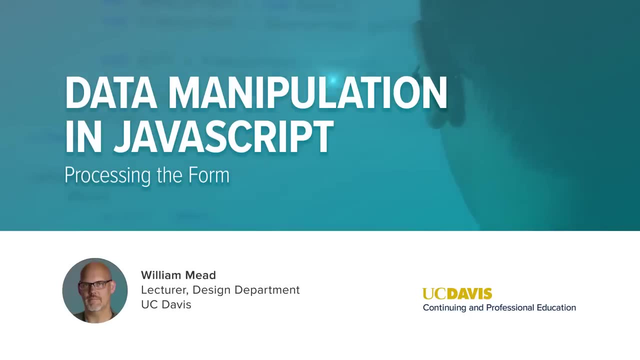 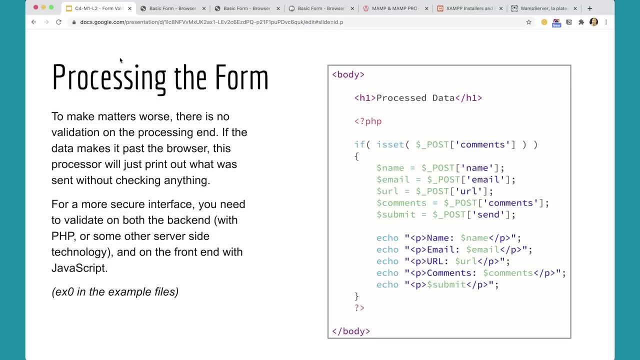 But you could put required equals, quote required, and that would work just fine as well. An important thing to note about the example zero files is that there is no validation on the back end happening here at all If you go look at the PHP form and this is not a class on PHP. 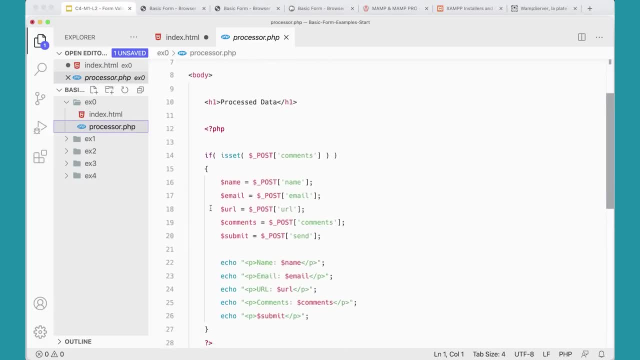 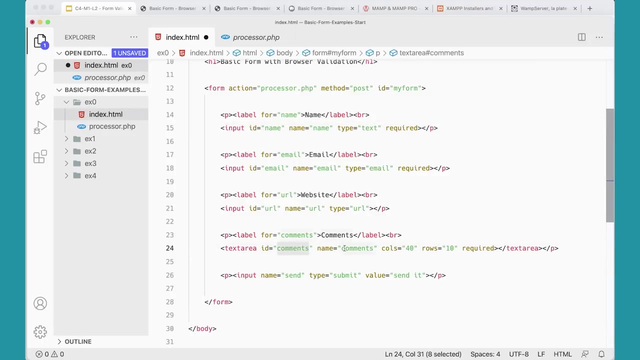 but it's worth mentioning this and looking at it. anyway, If we go look at this form, it's just checking to see if this field has been set, meaning has it been sent with this form over here? Has this field comments actually name? 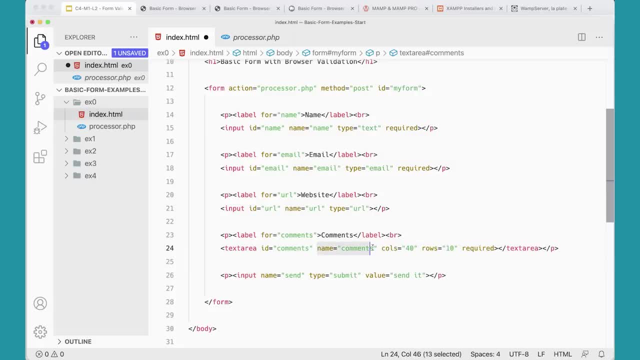 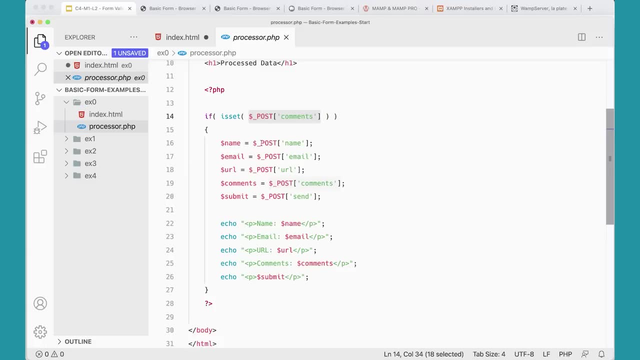 It's going by. the name. name attribute is what's required here. comments: Has that been sent over to this file? If it's been sent over here, it's just going to take the data that somebody typed into the field name- It's not going to check it or anything- and assign it to a variable name. 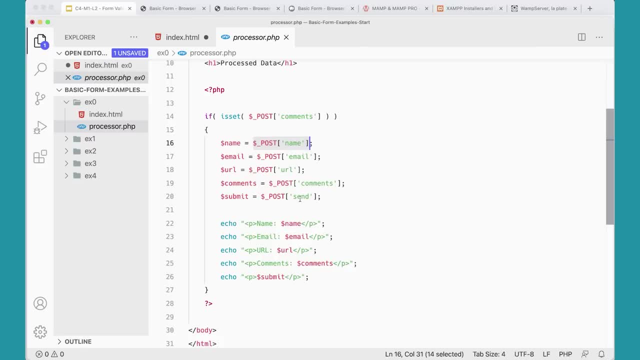 Same thing with the email, the URL, the comments and the actual send button. So the value that gets put into here- send it- will end up into this variable over here called submit. And then we're just echoing these things out and I'm just printing them on the page with paragraphs: the name: 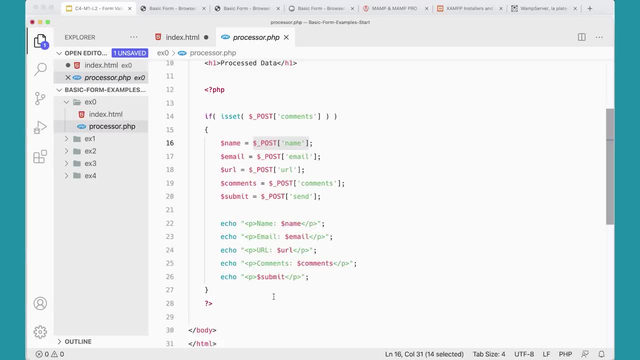 the email, the URL. So I'm not doing anything fancy with this data, but I'm not checking it either, And that's really a problem. You really have to make sure you do data validation on both the back end and the front end. 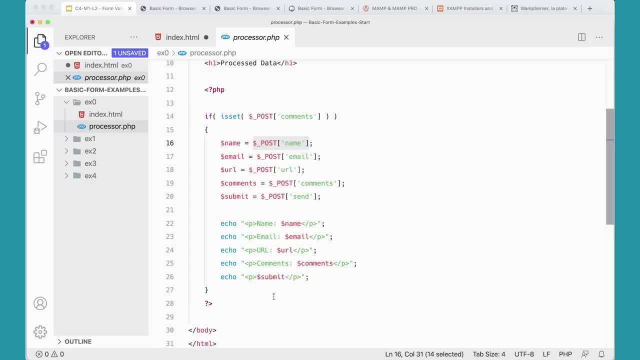 The back end validation is to make sure that people aren't submitting malicious data to your server. It's possible to send, say, a SQL statement in a field and then it's possible that on the back end that SQL statement could get processed as SQL and do bad things to your database. 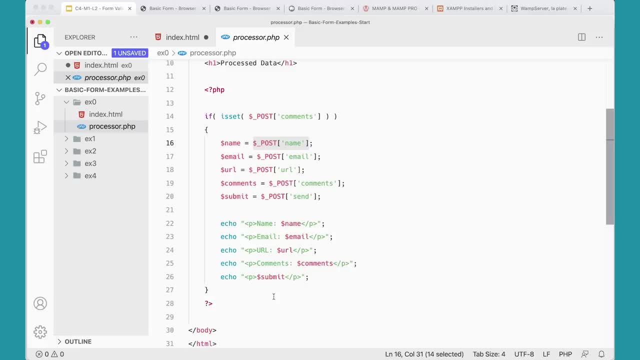 We're not doing anything with the database here, so there's nothing really bad to do. But you always want to make sure that you're doing validation on the server side, because you can't count on somebody's browser having JavaScript turned on or something like that that could be controlled on the front end. 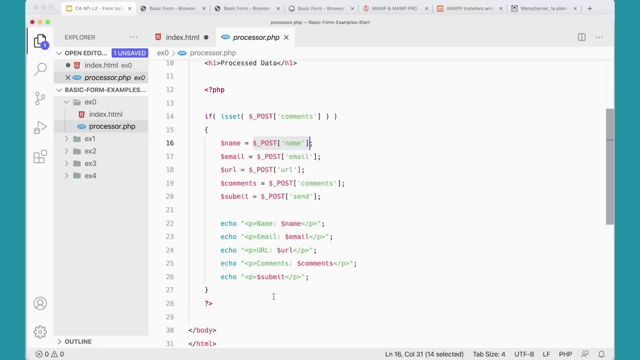 So you want to make sure that you're doing validation on the server side. The front end validation is really for the user and for helping the user fill out the form properly And it's for them. So back end validation is for the site owner or the product owner. 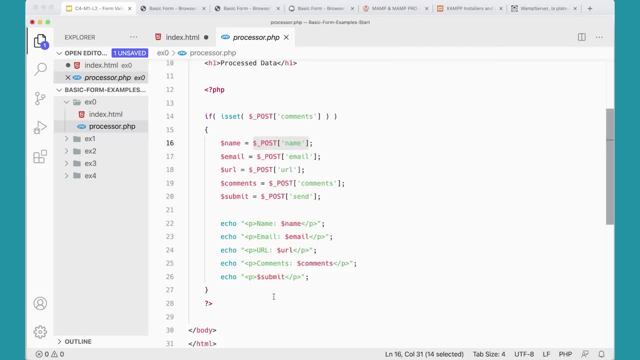 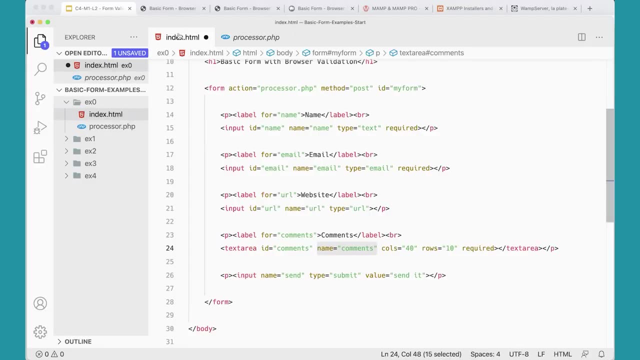 And front end validation is for the user, And that's really, really important. It's also important to note that if you were to take this file, this indexhtml file, just open it up in your browser directly, like this here I have it here. 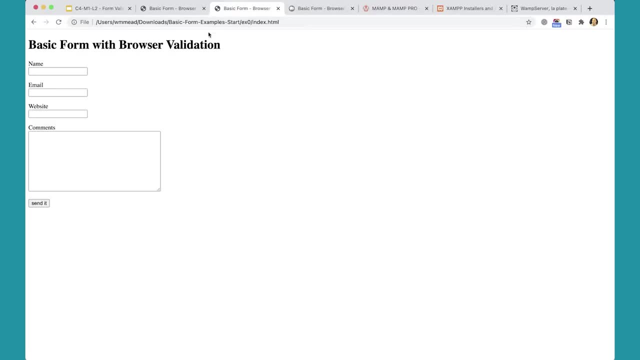 Open from users. you know from my web page, from my desktop here. If I fill this one out, Let's skip the website- and I click send, I just get a PHP file, and that's because PHP needs to be processed on the server. 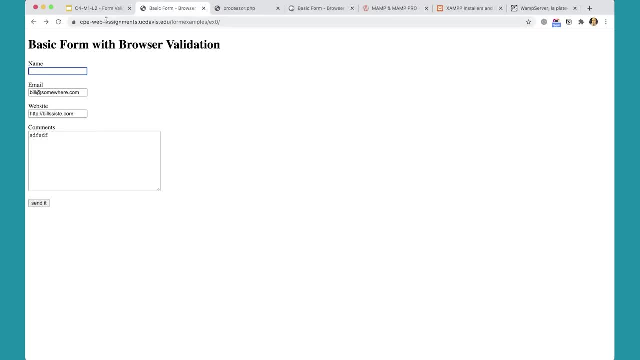 So that's why I provided these links: so you can test these out on the servers. These are on our server here, But if you do open it locally and test it, it'll go through, If it goes through to the processor, if you get the JavaScript right and it goes. 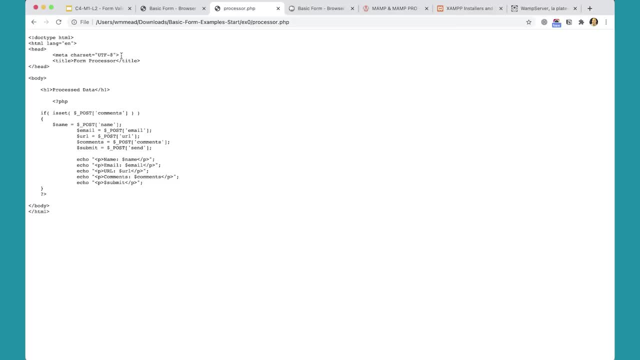 through to the processor. if you get the form validation right, it goes through the processor. you'll just get a PHP file And, honestly, for these lessons, while we're playing around with this, that's just fine. It's just notice that when you see this, if you're seeing PHP here, 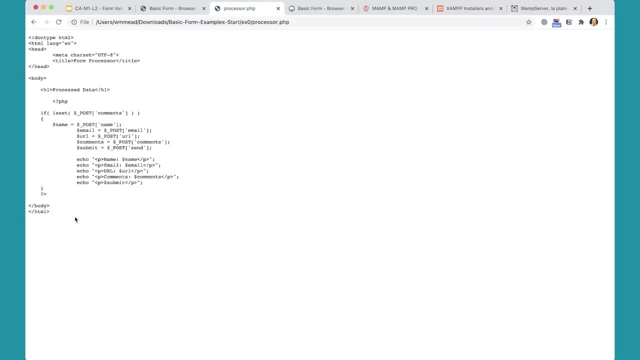 it's just because the browser says: oh, that's PHP. I don't know what to do with that. PHP should be processed on a server. Another option, One, is to use a local server. So I have on my computer. I have MAMP running. 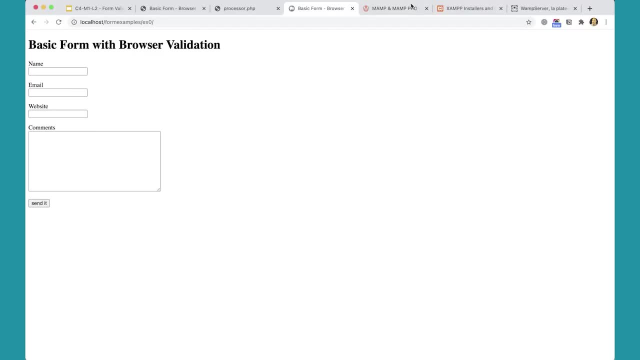 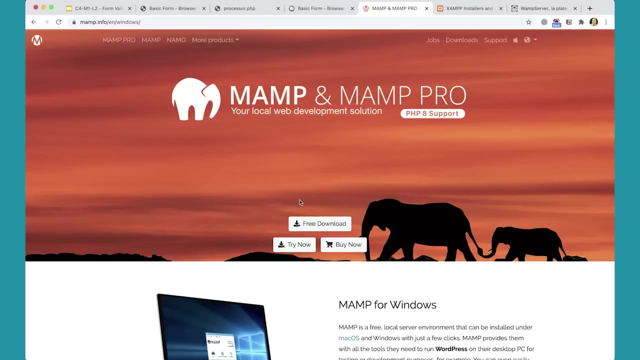 And this is that same file running locally through MAMP And you can go to MAMP and download MAMP and you can just use the free version. And they actually have MAMP for both Windows and Mac. It initially stood for Mac Apache. 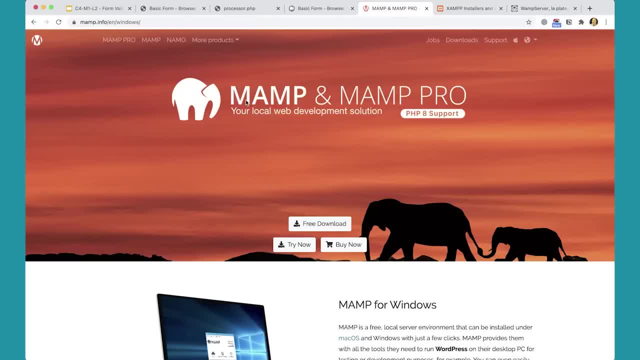 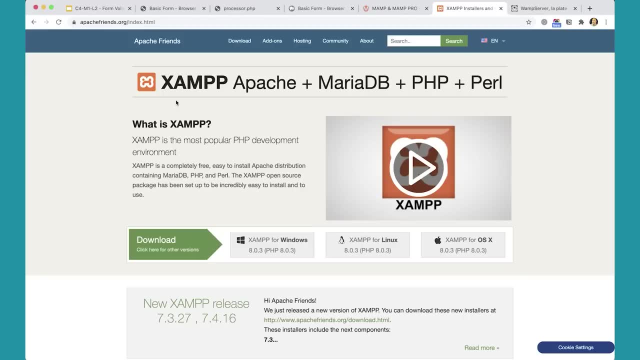 MySQL and PHP, But now they have it for Windows As well, which doesn't really make sense. Another alternative product you could use is XAMPP, which they have a version for Windows, for Linux and for Mac OS, So you can- you can- download XAMPP and try that one. 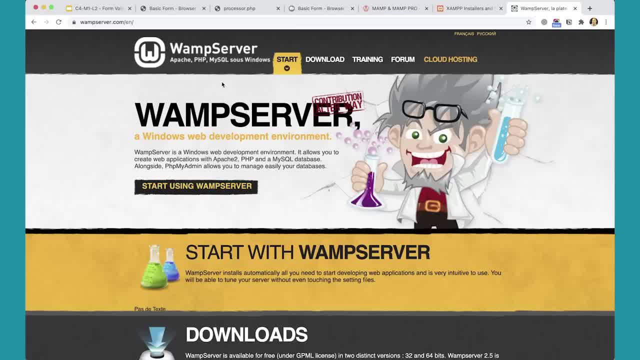 Or, if you're on Windows, you could use WAMP And all of these. the AMP stands for Apache, PHP, MySQL, And so you can run these on your local server. What does that look like when you run it on your local server? Well, when I installed MAMP- 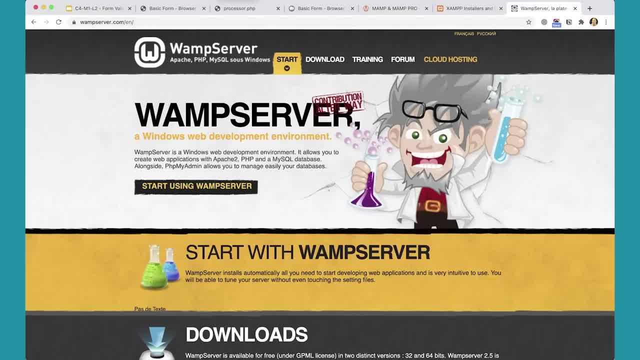 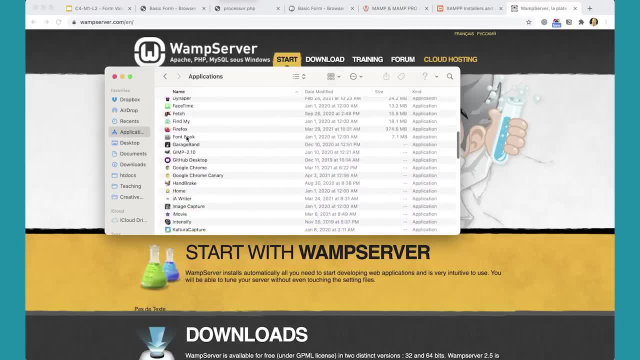 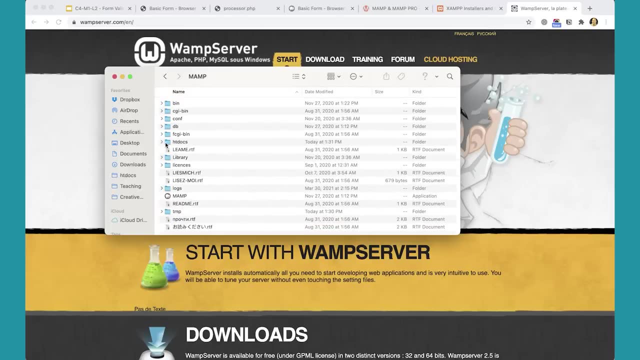 I have in my hard drive in my applications folder. I have MAMP installed here. If you go down and look through here and find MAMP here, it is here, And inside MAMP is a folder called htdocs And I took those same files that I downloaded and I put them here form examples. 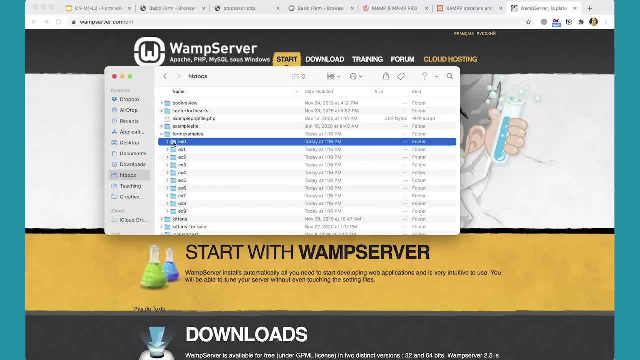 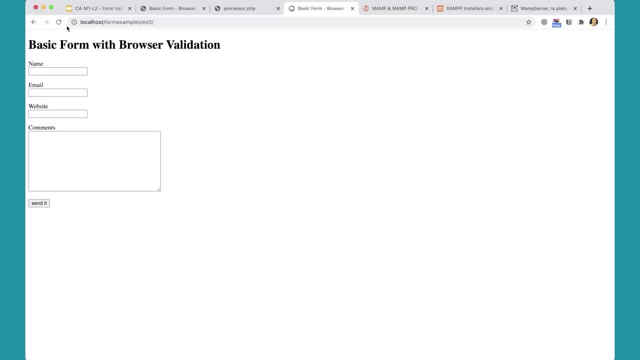 So these are the form examples we're going to look like, look at, And here's example zero. So by coming over to here with MAMP running, when I run MAMP it looks like this: This is MAMP running. I click start here and then it says stop up here. 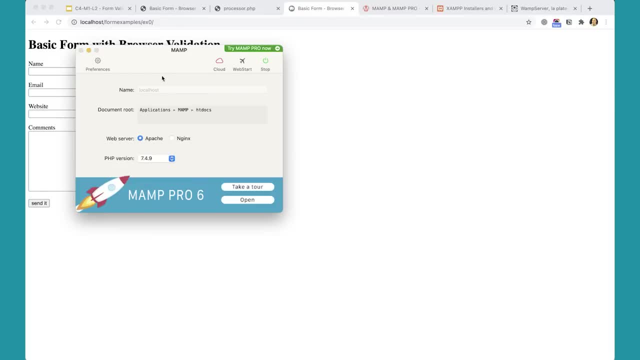 With MAMP running I can go to localhost. I have set, I've changed the, I've changed the ports so that it uses the default ports here- 80 and 80, rather than the MAMP ports. But if I just go to localhost, 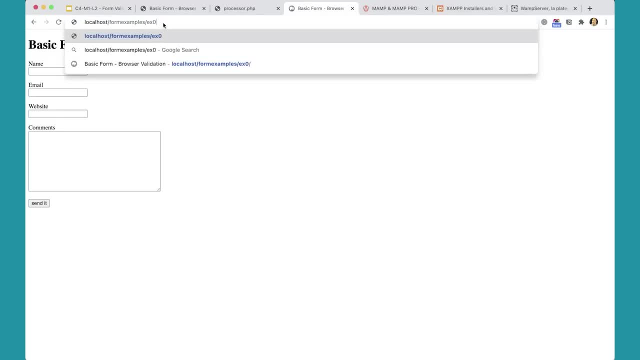 what I see is just go to localhost. I'll see all the files that are in that htdocs folder, that are inside the MAMP folder In my applications folder, And I can click on form examples and load up example zero here. 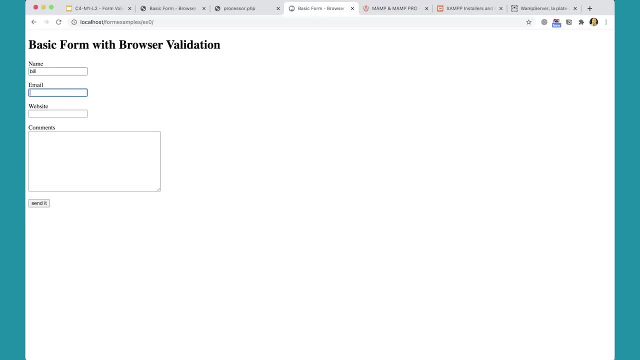 And I can fill this out And now it will work because it's going through the local server, The website, And you can see that's actually getting processed and working again. So the PHP is actually working because I'm going through localhost, I'm going through my local server and you could set up any of these applications. 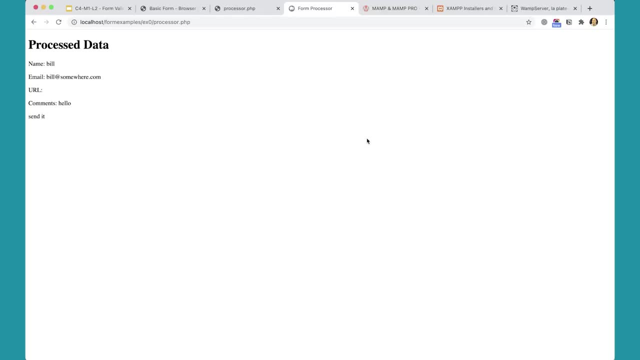 to run on your desktop if you want to, but it's not really necessary, because if you do it, if you do it just from the desktop, you'll just go through and you'll see the PHP file show up And, honestly, we're not really going to do a lot with server side validation here. 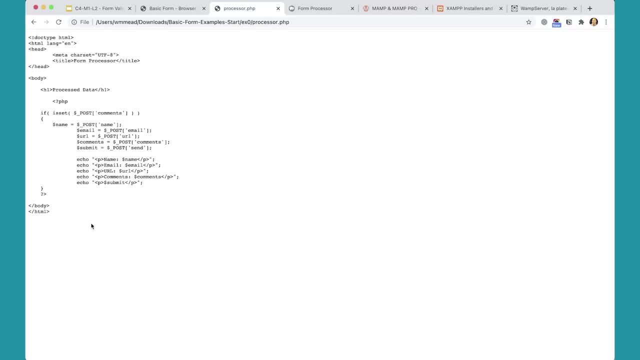 I just want to introduce you to it, so you're aware that you have to have it. But we're going to be focusing on the actual front end browser validation on the front end and working with that, with the built in validation that's built into the browser: JavaScript validation, jQuery validation. 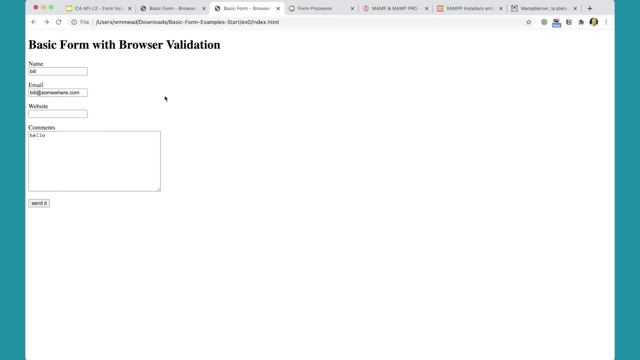 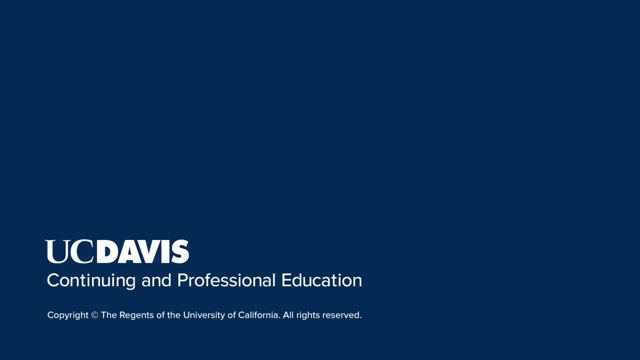 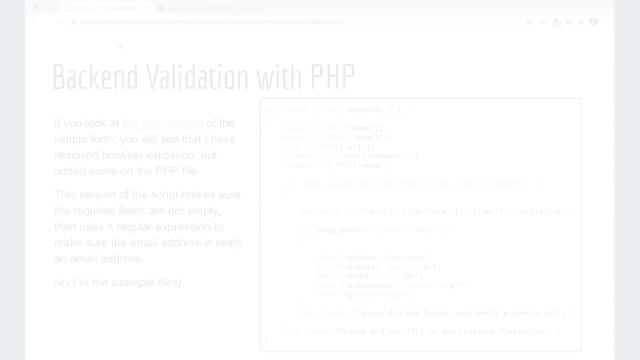 as well as a jQuery plugin that will do validation. So we're going to really be focusing on the front end, But it's important to note that you have to have back end validation as well- Back end validation with PHP in the next version of this file. 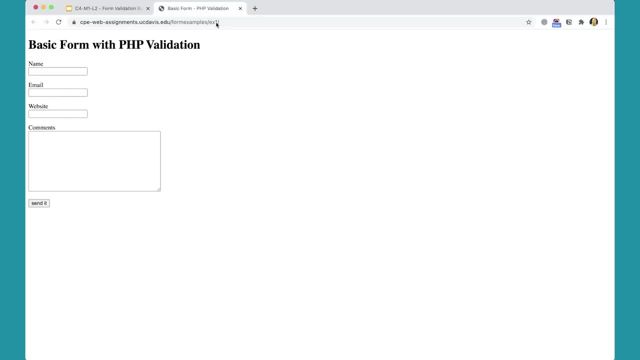 And I'll provide this link for you, but it's just basically EX1.. We have the same form, but this form doesn't have any front end validation. I've removed required from here. Instead, we're using validation on the back end only for this one. 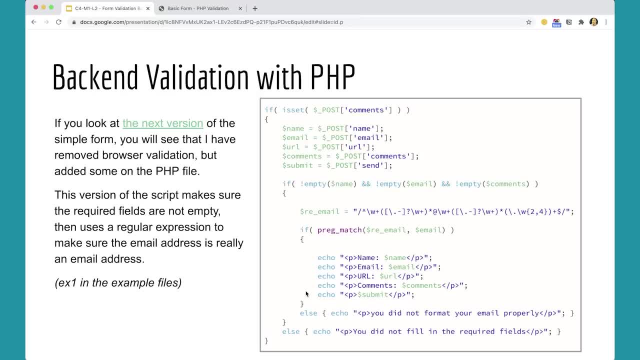 So you can see what some of that back end validation might look like. and this is just simple back end validation. We're not doing anything too complicated here, But if we come over and look at this PHP file, it's worth taking a minute for it, even though this isn't a PHP course. 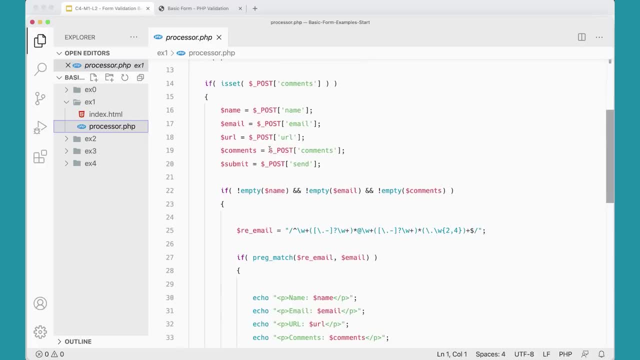 It's worth understanding that this validation is happening on the back end, So the same thing happens as before, in that the script doesn't run unless the form has been sent to the processor, And when it is sent, we go and we assign the values that somebody typed into these fields that match the name attribute. 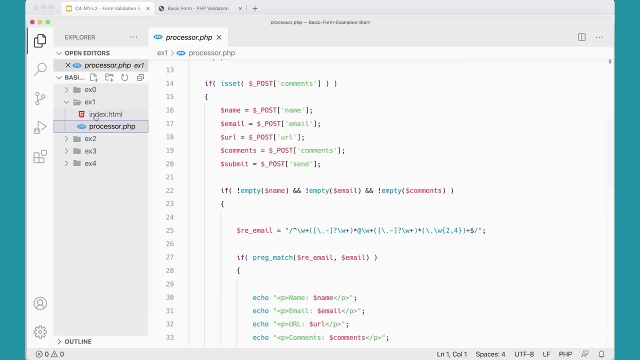 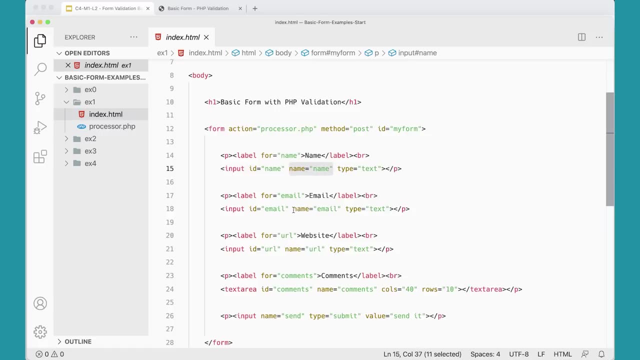 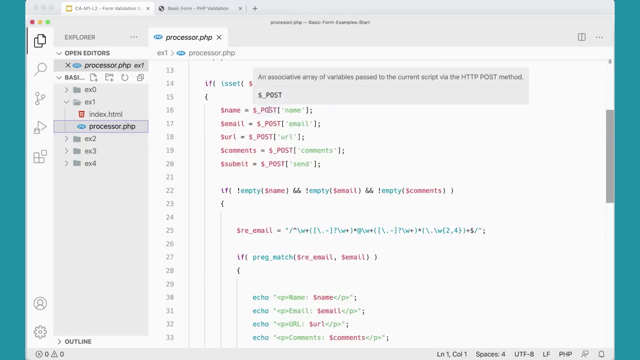 Again, post name is going to match the field over here that has the name attribute name on here, And post email is going to match the name attribute that has email over here. So you have to have those attributes in your fields, in your inputs over there. 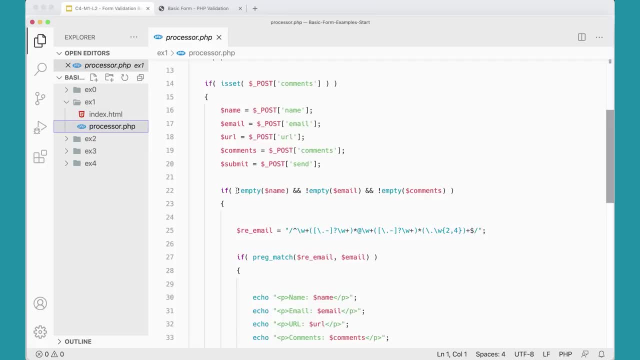 URL comments sent And then it's going to check to make sure that the name is not empty, The exclamation point or bang empty means not empty and the email is not empty and the comments is not empty. The URL is optional, so that can be empty if you wanted it to be. 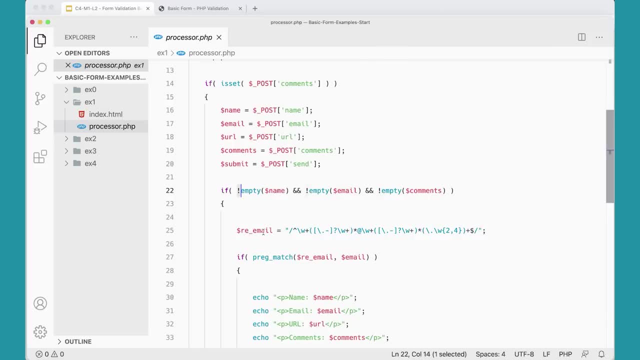 And then we're going to check to make sure that the email- this is using a regular expression. we'll talk about regular expressions more in a minute, but it's checking. it's using a simple regular expression to check what somebody typed in the email field, to make sure that what they typed. 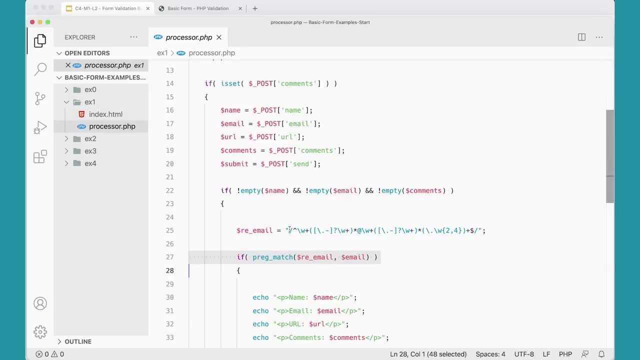 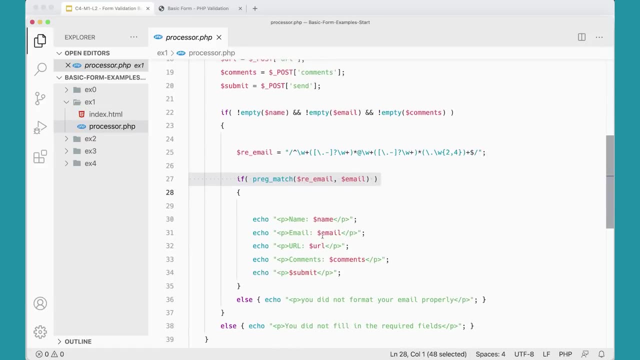 into that email field matches this pattern for what an email should look like? If it does, then we're going to print this stuff out. If it doesn't, then we're not going to print that stuff out. We're going to echo out one of these errors. 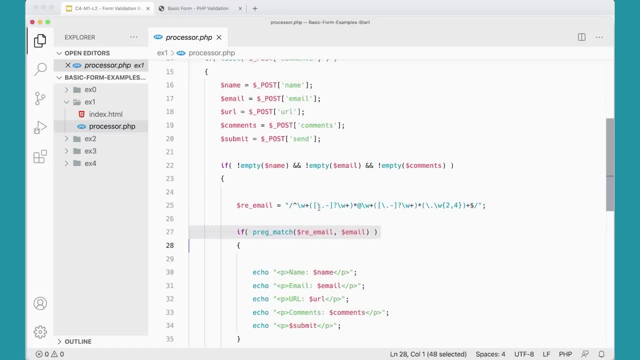 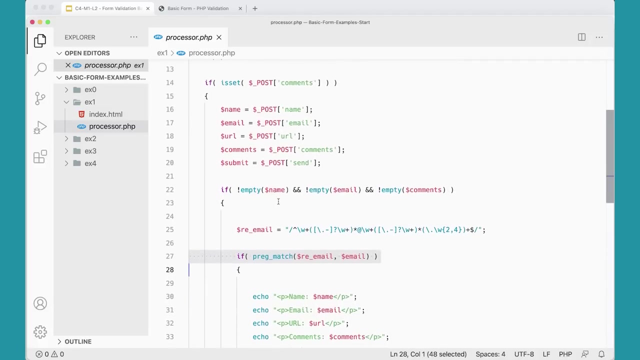 So we could do more. We could have a regular expression for the URL to make sure that it's actually a URL and make sure that that passes if that's been passed in. But this is enough of a back end back end validator to just check the back end. 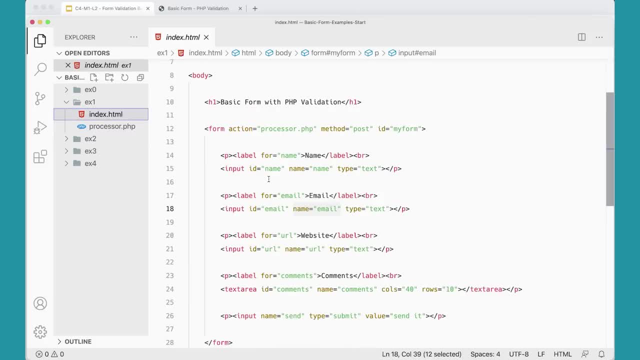 So let's go see what that looks like, because on the front end you'll notice, I've removed the required from all of these so that we don't have any, so we don't have any, Any validation going on here on the front end at all. 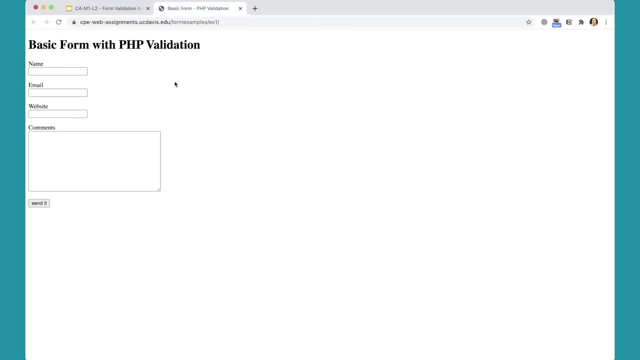 And we're just going to test it on the back end. So let's see what happens over here. If I just click send, it it's going to say you do not fill out the required fields. So essentially We click send so it got the comments. 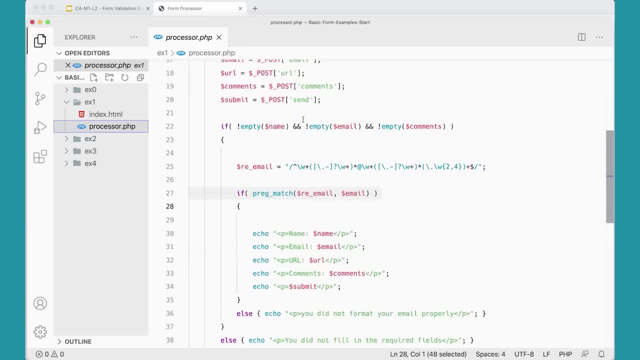 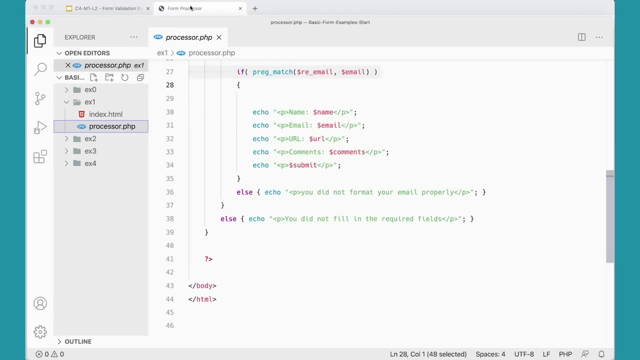 That comments thing came through but it was empty. And since it was empty, this else statement fired down here. You do not fill in the required fields. Let's try it again and see what some of the other ones are. But this is back end data. 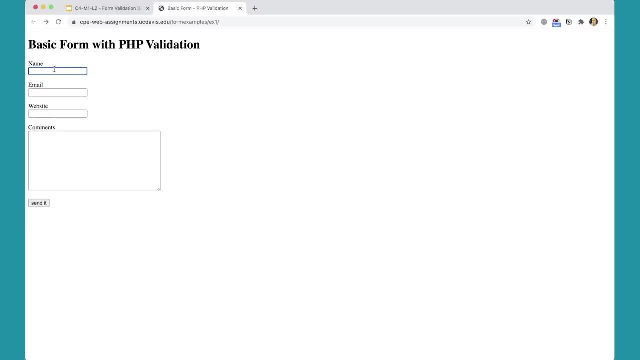 verification sort of in process there. So if I put Bill and I put a broken email address in here and then a comment, you'll see that it will say you did not format your email properly. So you can see that this back end validation is in fact working. 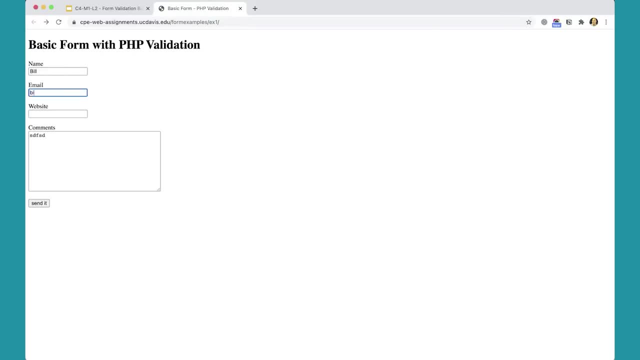 It's not very sophisticated but it is. It is working. Bill at some player dot com. And then again I could put gobbledygook in for the website. I have not really checked that and then that will go through And you can see this is bad data here because I haven't actually checked for that. 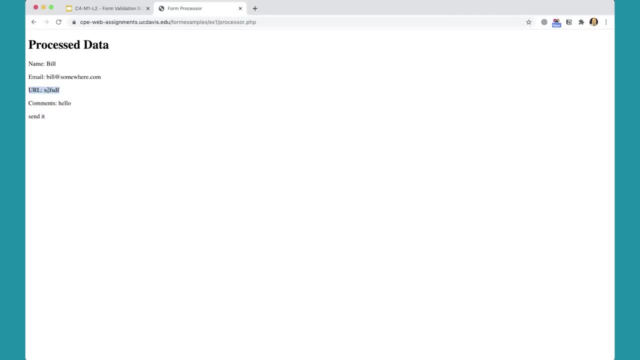 But this is enough of a validator for us to be getting on with for the back end for the rest of this lesson. If you were doing A real something real on the Web, you would want to expand the script considerably to make sure the URL is checked and 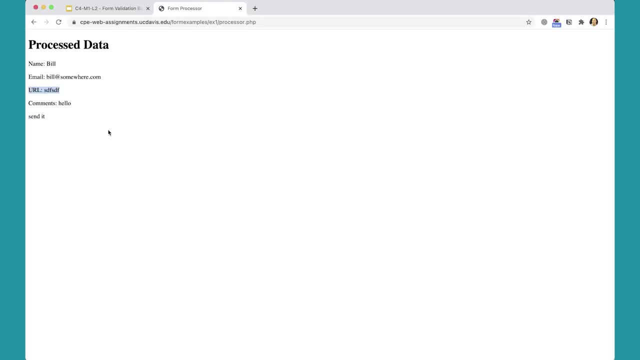 any other data. it won't allow any other bad data to get through. You might want to make sure that it's only letters and only letters and apostrophes. You know you put a regular expression for a name up here, or regular expression. 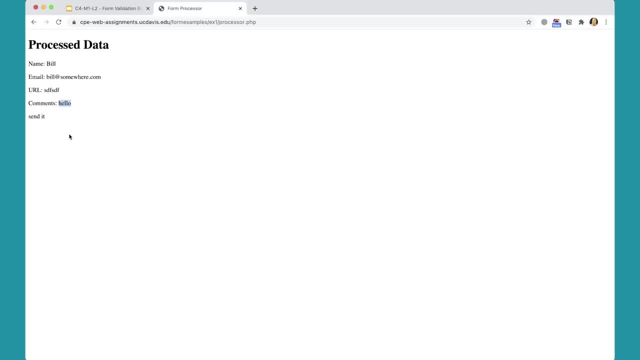 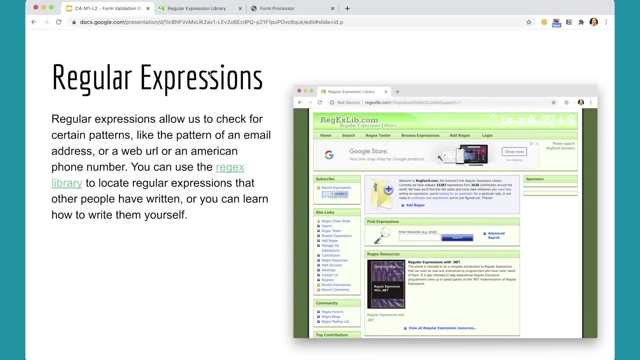 Make sure that you don't put in weird content down here as well. If you're doing stuff with the database, you have to do a little bit more to even sanitize it, even a little bit further For regular expressions. if you're wondering where I got this thing for the email address and how do you come, 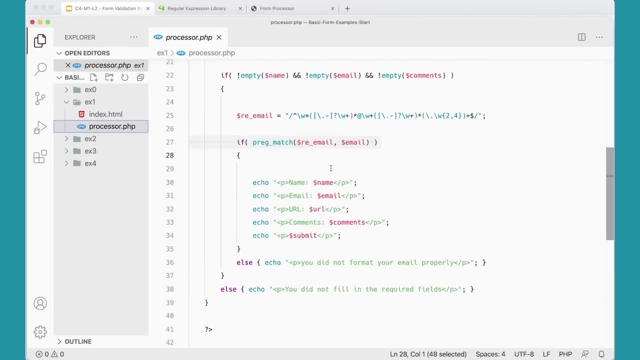 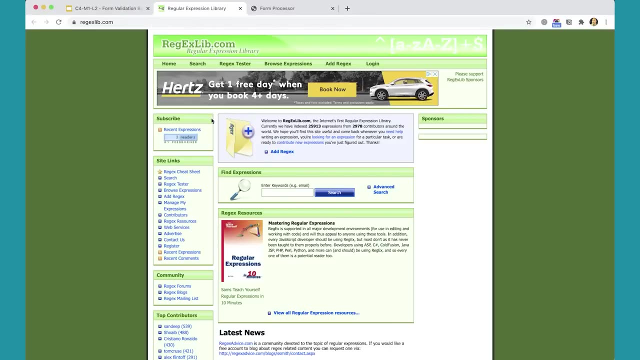 up with that you can actually go to a website to to get things like this sort of regular expression here, And you can go to this regex, regexlibcom, and look up regular expressions. So, for example, if you said you know: 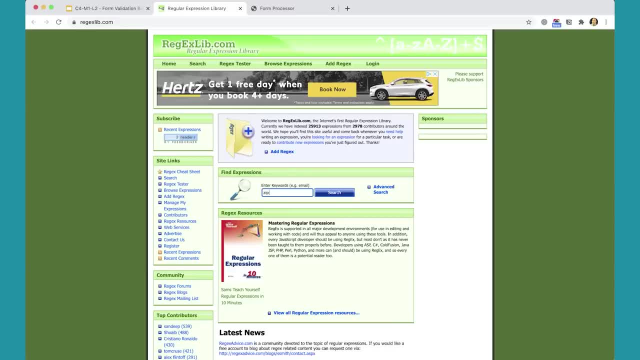 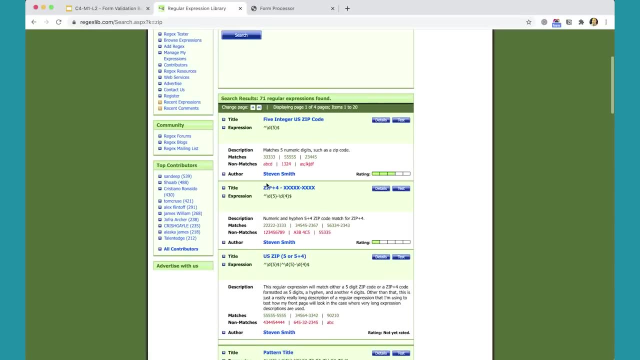 I really want to make sure somebody types in a zip code properly. I could look up a zip code search and I'll find a number of regular expressions that I could use. So this one here will check to make sure that I've got five numbers followed by a dash and then four numbers. 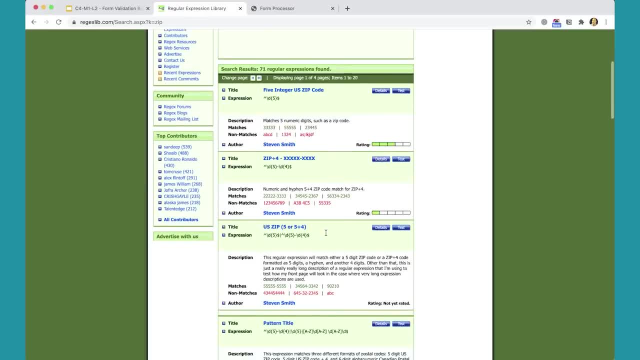 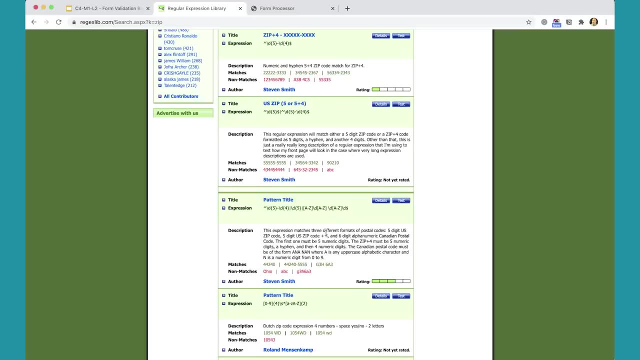 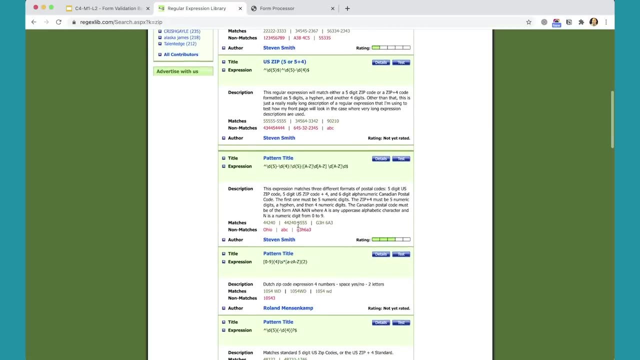 So these will pass, but these will fail. And you know, depending on where you are in the world, you might allow different types of things for zip codes down here. These will pass, but these will fail. So depending on where you are and what kind of regular expression you need, 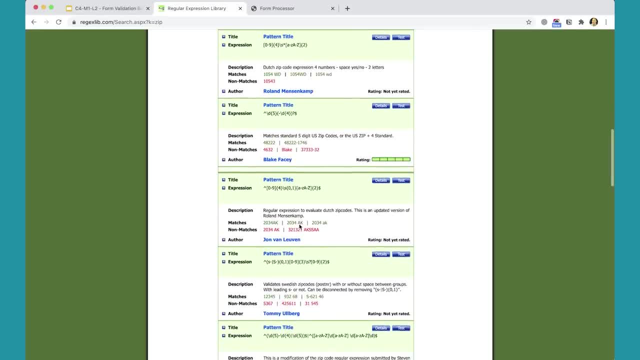 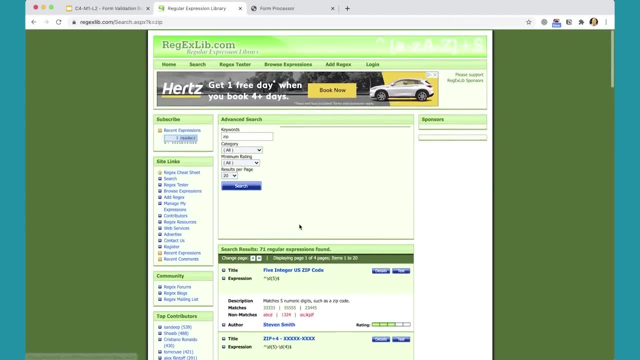 for your users. you could go and find a regular expression here. This website has been useful for a long time for this kind of thing, And there may be other places where you can go to to get regular expressions without having to write them yourself. 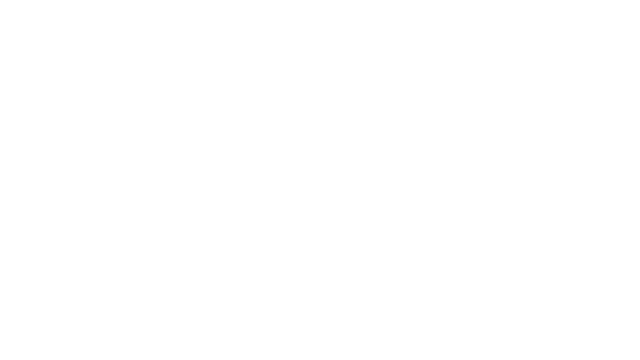 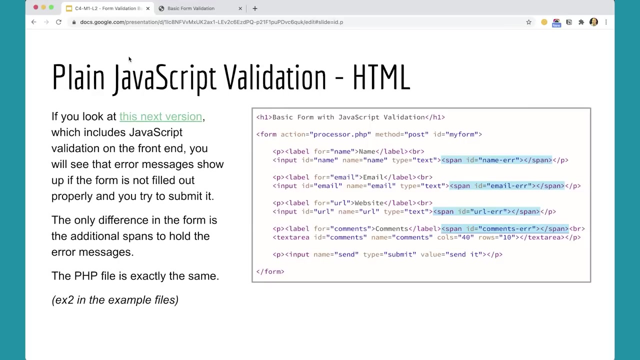 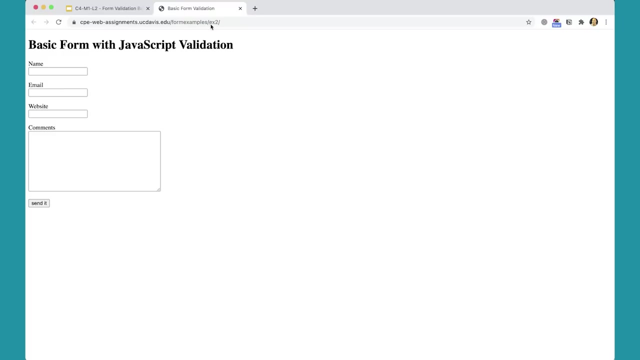 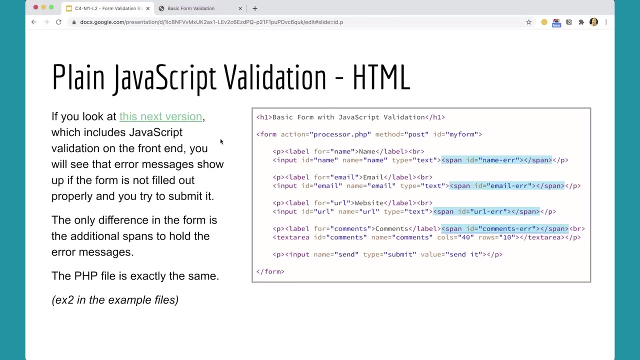 The next version of the script that we'll look at, which is in the EX2 files here, and I have it pulled up here, so it'll be EX2 at the end here. In this version, we're using old school JavaScript validation rather than the built. 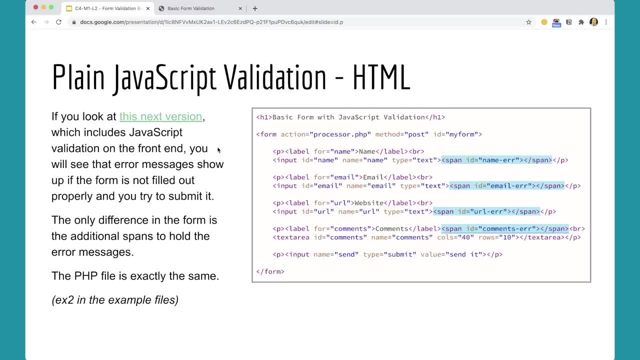 in validation. It's built into the browser by adding the required attribute. Instead, you'll notice that I've added spans with IDs and they're empty here and JavaScript will fill them in. Let's go ahead and give and try this out, just to see what happens. 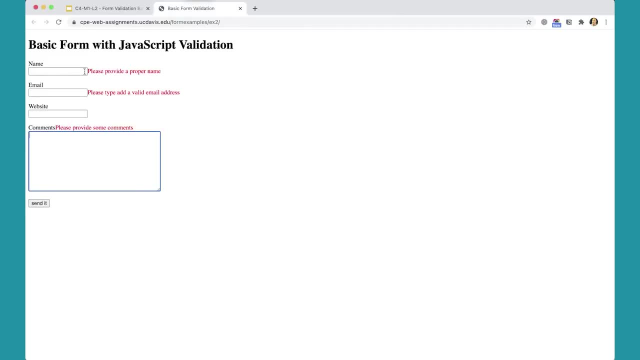 If I just click send down here, I'm going to get some error messages coming up telling me that I need to fill out the form. But if I fill these out, if I fill that one out and click send, I'll just get these. 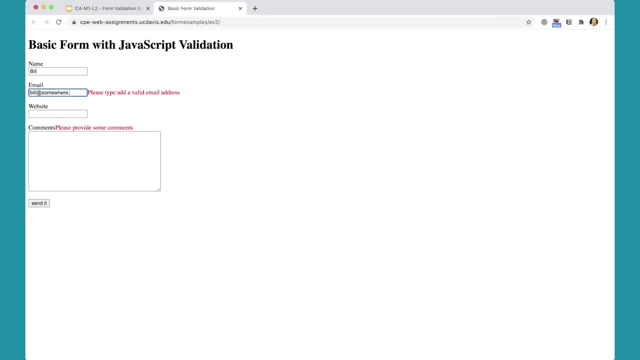 So I'm going to go to my site at somewherecom and I'm going to put in a bad website. I'm going to put in hello and click send. Now it says type a valid URL in the form of that sort of form there. 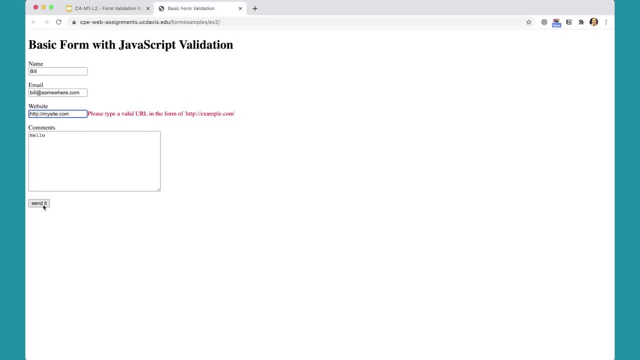 My site dot com, something like that, And then it'll go through and it will give me back my data. that has been processed by the processor. The processor file in this version has not changed, So if we come over and look at this, 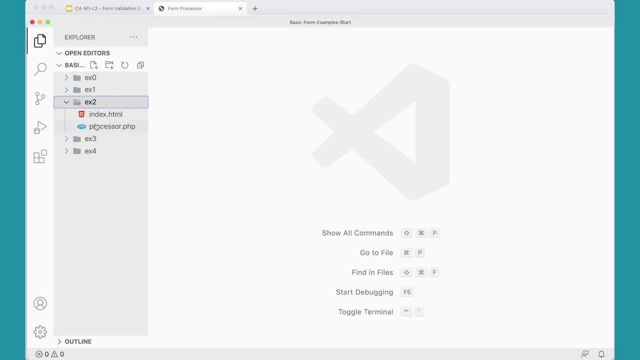 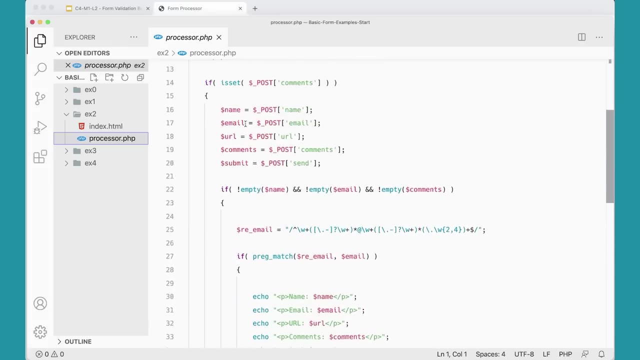 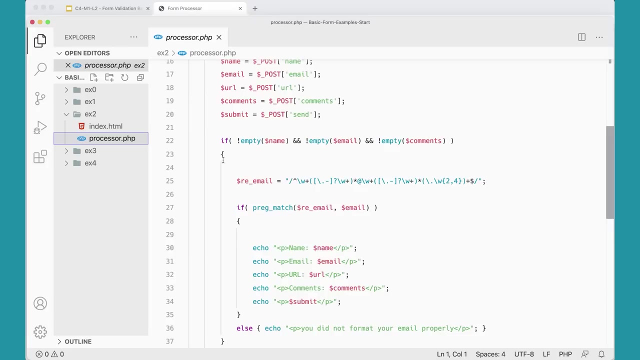 I'm going to close that and close that and look at example two. The processor dot PHP is exactly the same as the one that we had in the previous example, And the rest of these examples will have the same processor file because we're not focused on back end validation. 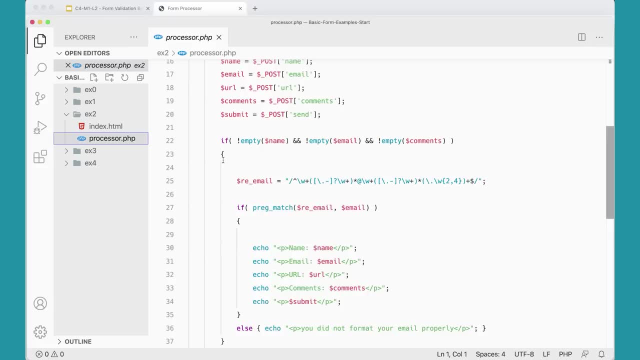 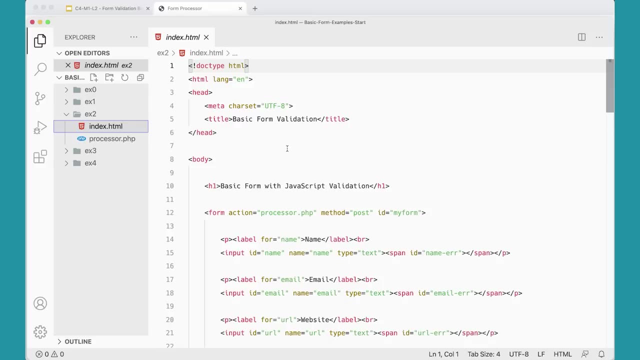 It's important, you have to have it, but we're going to be focusing from here on front end validation. Now I'm not having you type the front end validation out for this example, because it's kind of old school to do it this way. 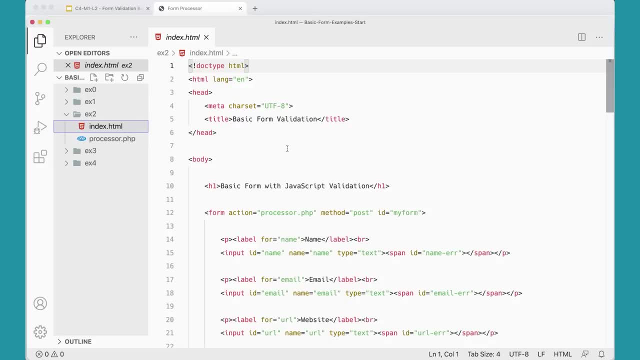 And there are more modern, better ways of doing validation. But I still think it's important to see how this works and what the strategy is here, so you can understand it and understand sort of where front end validation has been and where it's going. 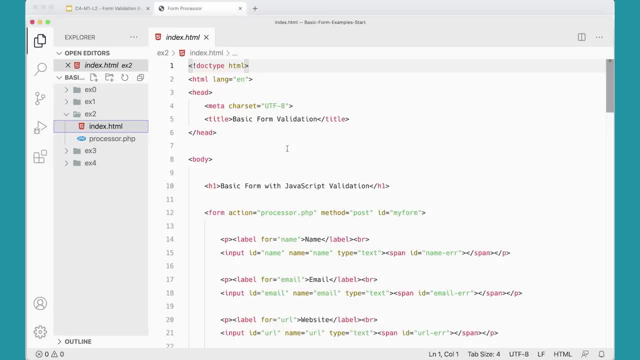 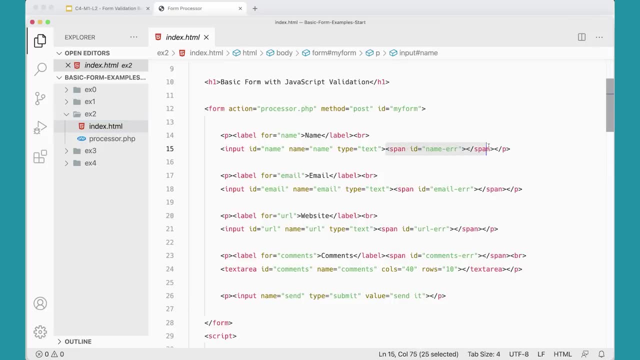 So you get kind of the scope of the whole sort of history of front end validation here And you can see again. I've added these spans which are currently empty. A span is just a generic element like a div, but it's an inline element. 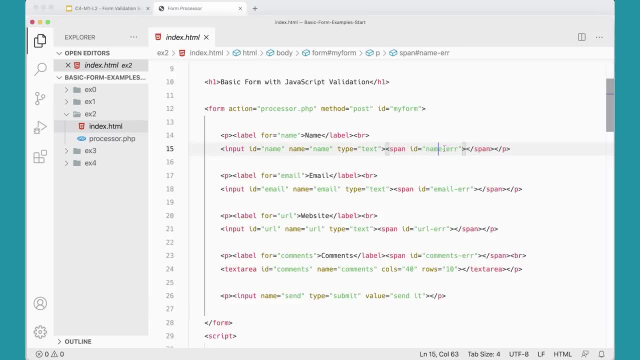 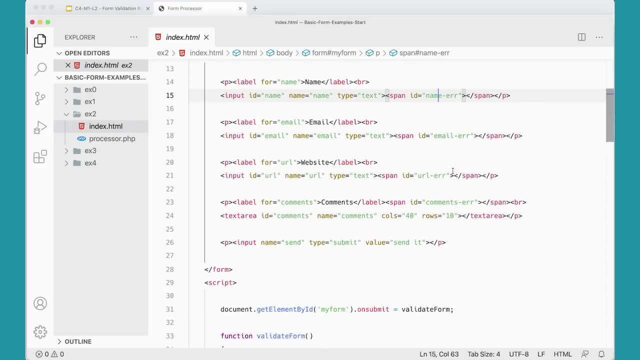 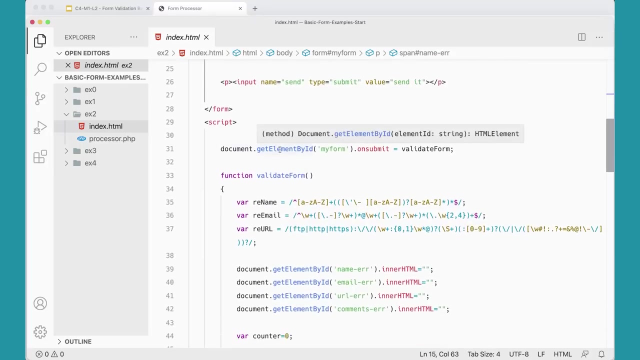 Notice that the ID is the name of the field with dash ERR for error on it. So it's that same name with that down there. That's important to notice. Down here I have an event listener that's saying document get element by ID. my form on submit. 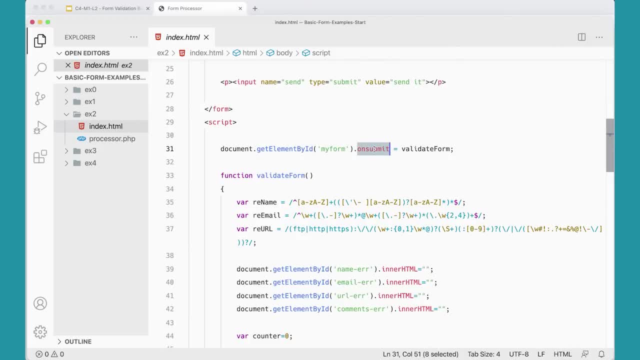 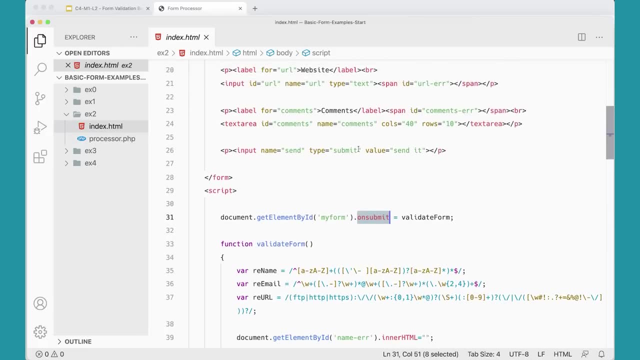 I'm using the on submit property to capture when the form is submitted. So this form is submitted when somebody clicks this input button here and then it runs a function validate form, and down here I've got validate form. I could use an event listener here, but I'm using the on submit. 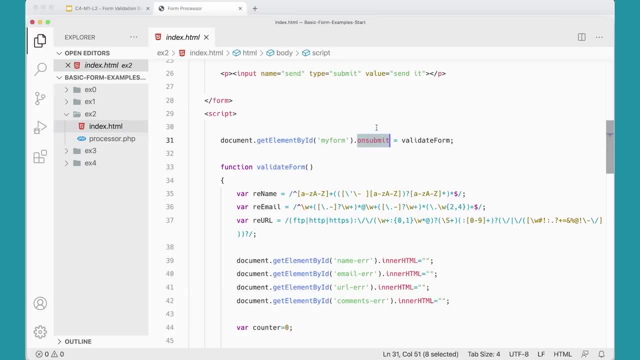 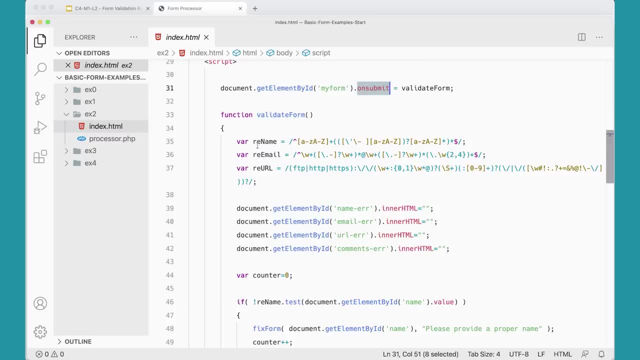 special event property instead. It's a little bit old school, but it's perfectly fine. It works perfectly fine. Down here I've got a validate form and then I've got some regular expressions. I've got a regular expression for names, which will allow letters and apostrophes. 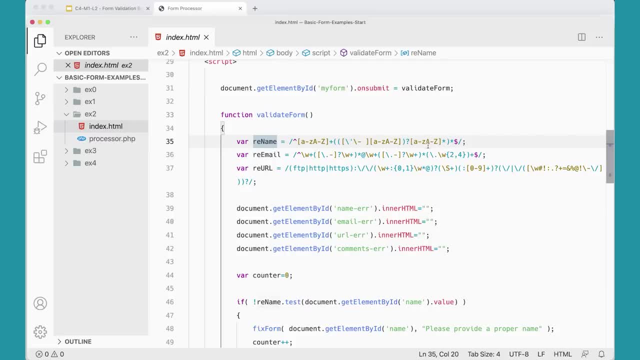 and dashes uppercase or lowercase and that's it. So you couldn't do a name with the number in it or something like that, or a weird character or something like that. that won't pass this validation. So be careful what you name your kids. 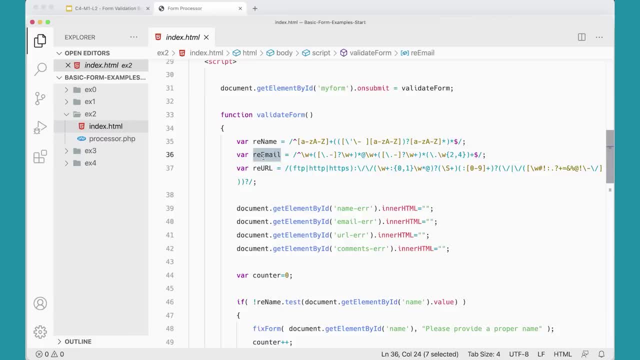 And then and then an email address. Again, this is the same regular expression I used before. This regular expression is perhaps not up to date with some of the newer domains that are available out there- top level domains. I think I'd run into problems with this regular expression. 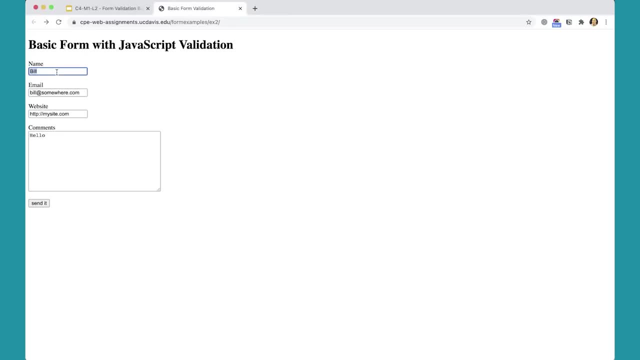 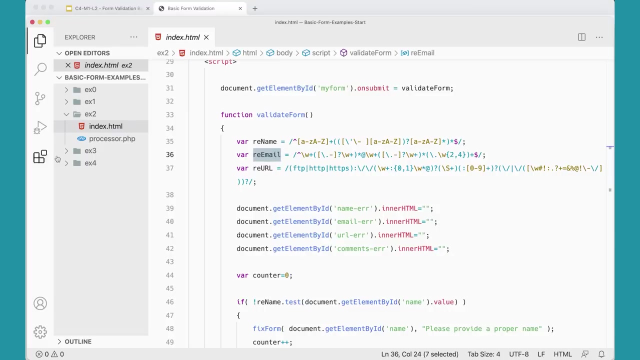 If I used something like Bill at somewheredesign, I have a feeling, yes, it's not going to like that because this is a new top level domain, So you'd have to go find a regular expression that would allow that. But for our purposes today it's perfectly fine. 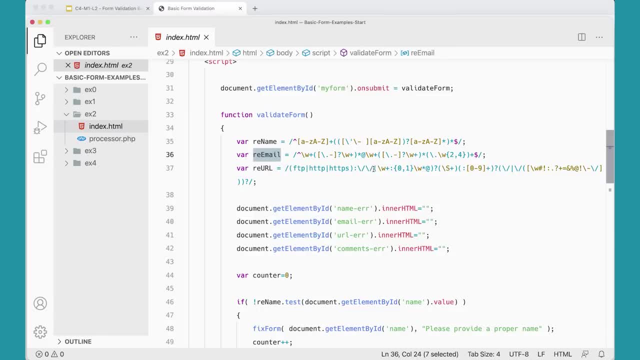 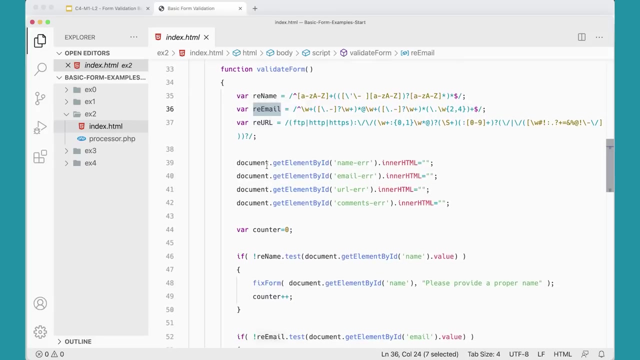 OK, and then I have a regular expression that's going to check for URLs- FTP, HTTP, HTTPS- And then you can kind of make out what it will accept here for URLs. So I've got these regular expressions get set up, and then I'm getting these. 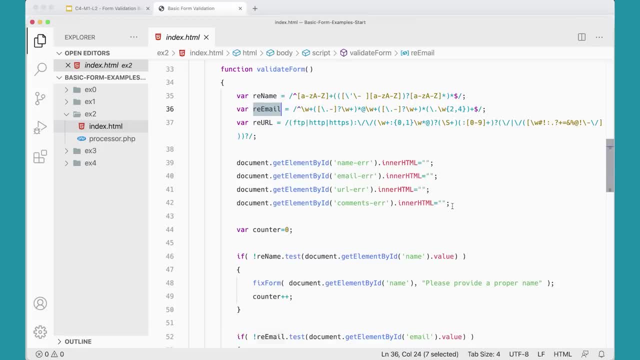 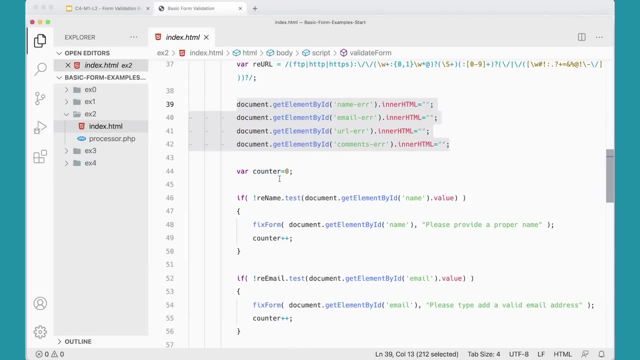 elements and I'm clearing them out, and I'll explain why we need to clear them out in a minute. but we're clearing them out and then I'm setting a counter, And this is the guts of the script. So the counter starts at zero. 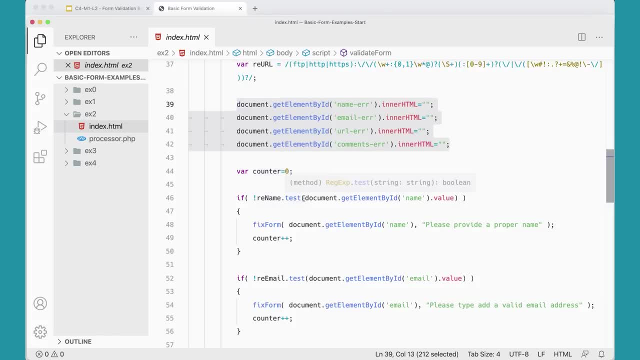 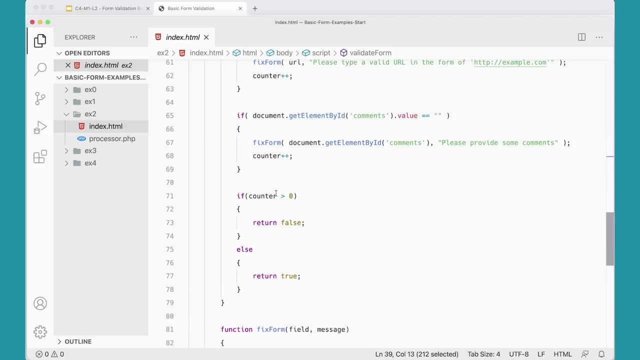 And if one of these fields does not pass, the counter gets incremented. So down at the bottom of the script, if the counter is ever greater than zero, it meant that one of the passes did not happen, and then we return false. and return false keeps the form from being submitted. 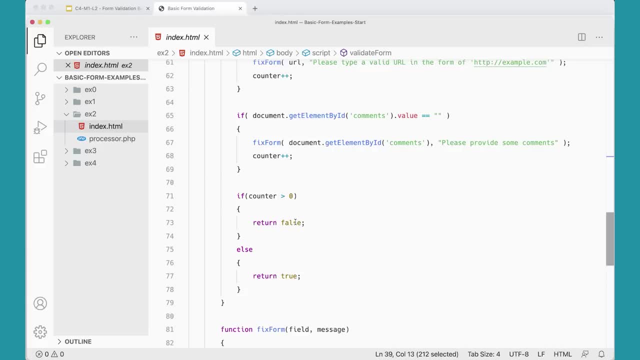 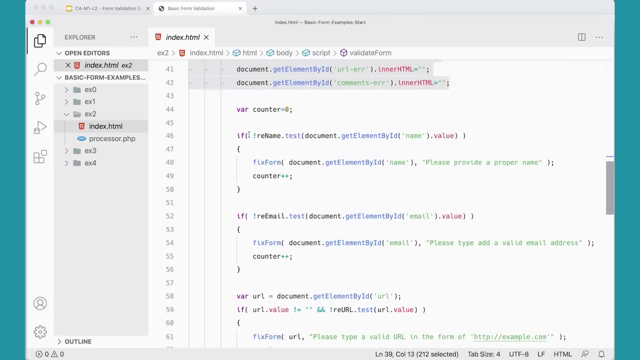 from being submitted properly. This is similar to using event prevent default, And we could actually update this to use event prevent default. This is a little bit old school here, and that's fine for this thing here. OK, so we're going to check each one of these fields. 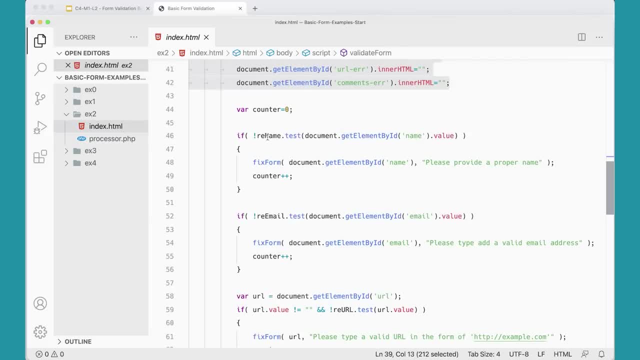 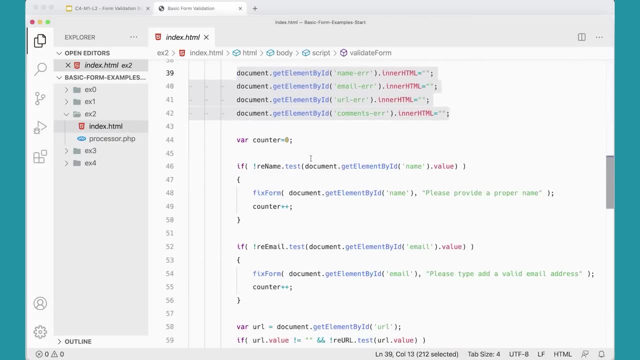 We're going to go and get the value out of the name field and test it against the name regular expression And if it doesn't pass, I'm going to run a function called fix form, which is down at the bottom, which gets the name, and then we pass in a message that we want to get printed. 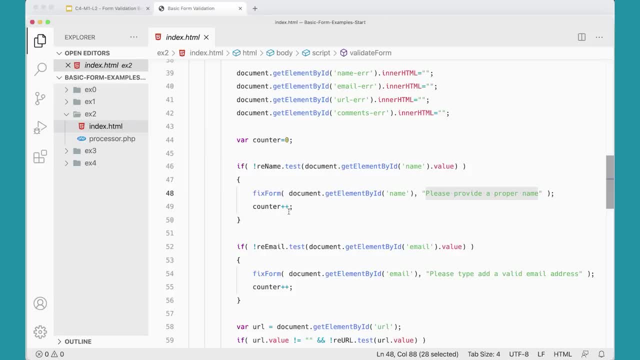 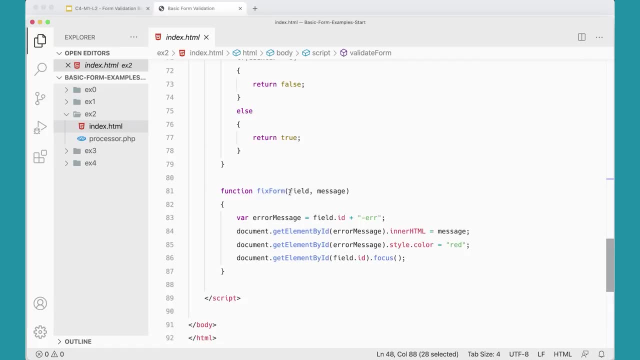 if it did not pass and the counter gets incremented. And again, if the counter gets incremented at all, the form doesn't run. So down here under fix form we say what field are we checking And what's the message we're passing in. 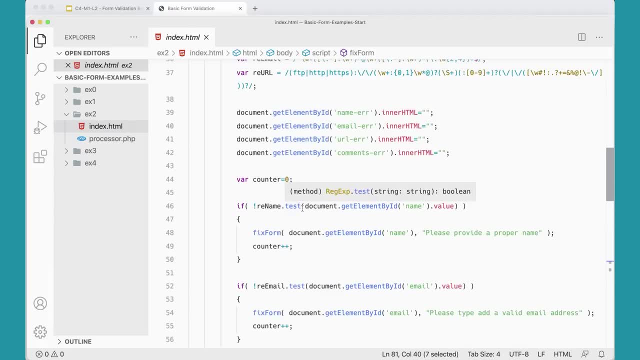 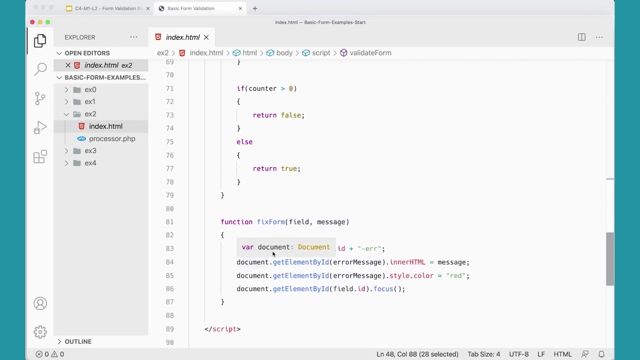 So up here for the name field, we're passing in this field And this message, we're passing that into this fix form function. So we're passing in the name field, in the name message, And then what happens is that we have a variable called error message. 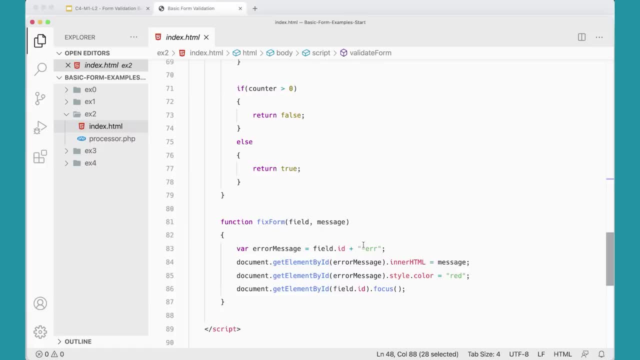 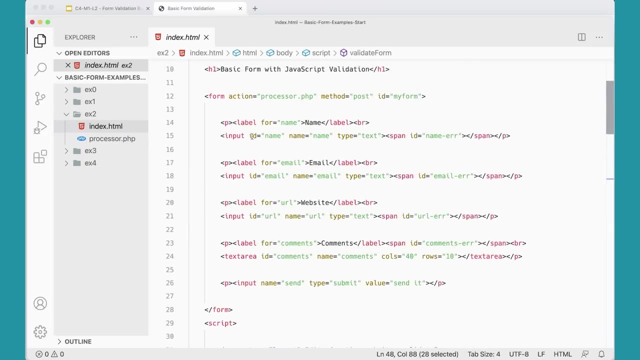 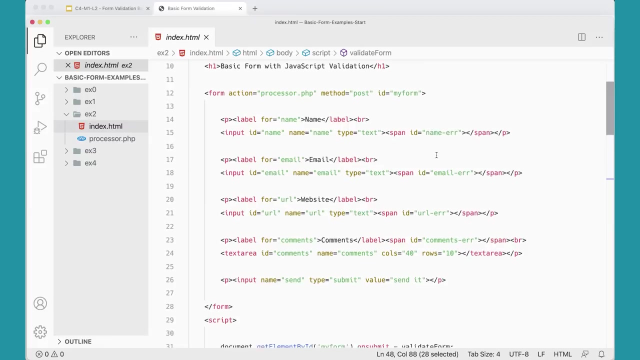 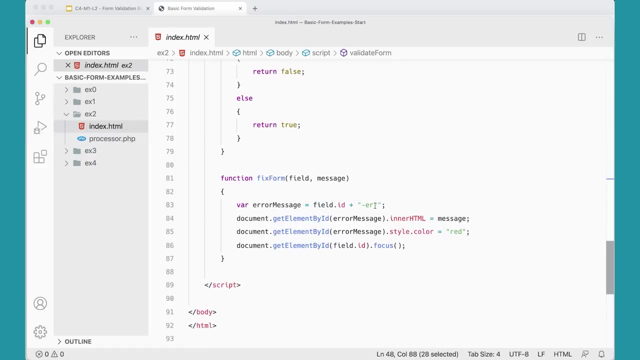 which gets the ID plus dash error, So the ID of the field for name up here. if we go back to our field up here, the ID is name plus dash error. So that's going to give me this name dash error error. So error message is going to be name dash error. 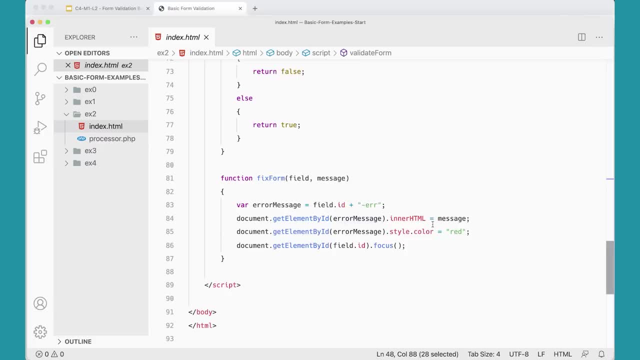 And then I can go in and I can set that error message in our HTML to whatever the message was. fill in your name and set in color to red. And I'm putting a focus on that field, meaning that the user, then the cursor, is put in that field for them to fill out. 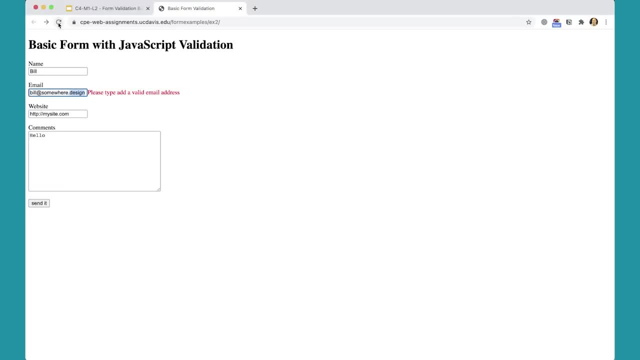 So let's go and test that out really quickly over here and just sort of see it again. So if I were to forget just the first name and put in an email Bill at somewhere, dot com- And I'm going to skip the website for now because that's optional- 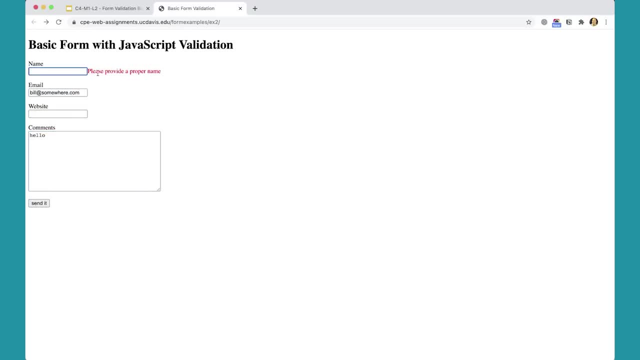 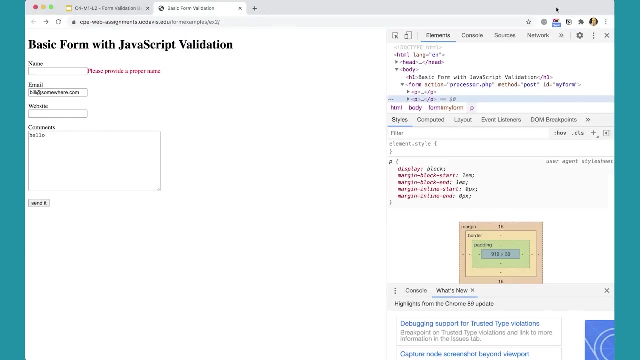 Hello, And then click send it. It says please provide the property setting that color to red And it's adding that that span. it's putting that in the span there. If I were to do inspect, You would see this down to the bottom. 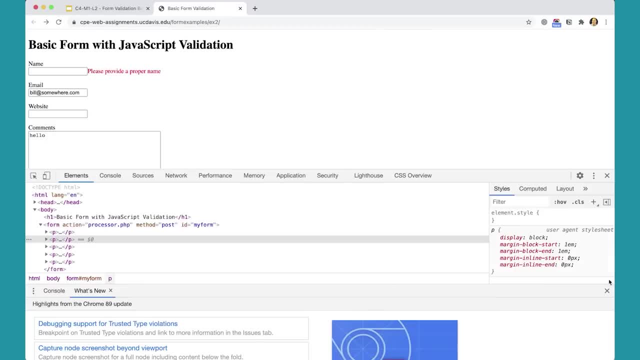 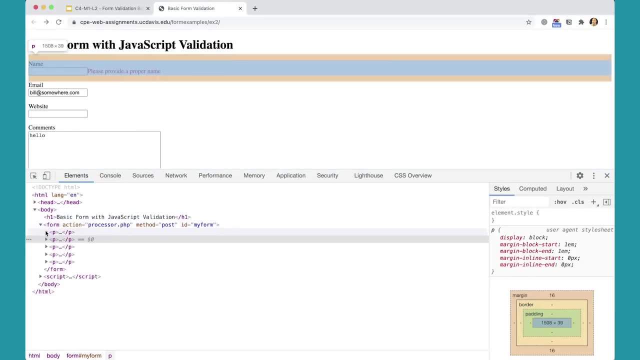 Here is that, and Look in here to This one. here you'll see that the span has added the style and it's added this message in here, plus the form has not been sent through because of the return false, So it's important to understand how that works. 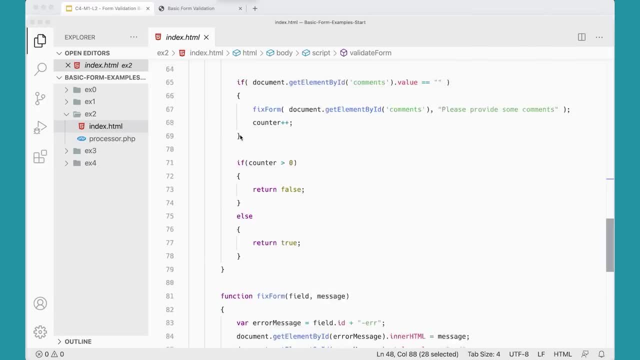 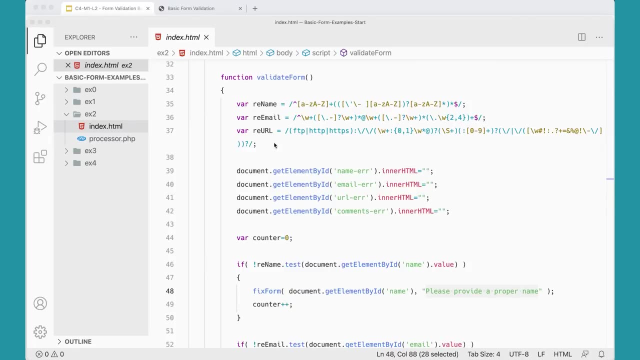 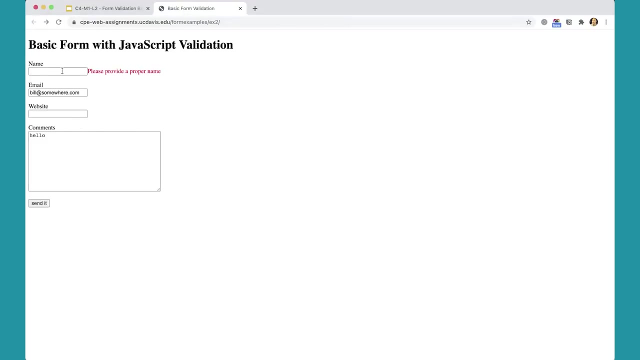 The last thing to clear up is: why do I have these, these things filled out here? And that's because each time I submit the form, I want to clear out any error messages and check it again and add error messages again. So if I put a name in here, 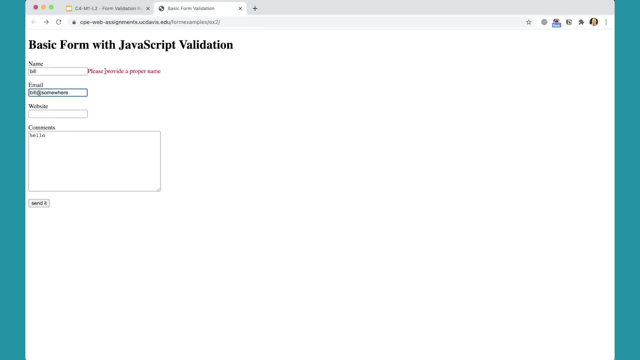 but then do the email incorrectly. I want to clear out this message but then add a message there so that message will clear out, And then when I run it and then it checks this one because this one's wrong If I didn't put that clear up there. 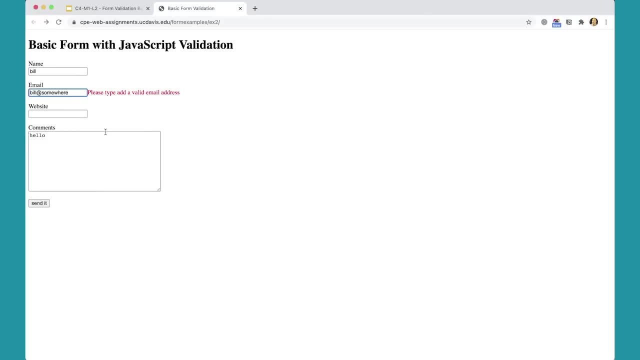 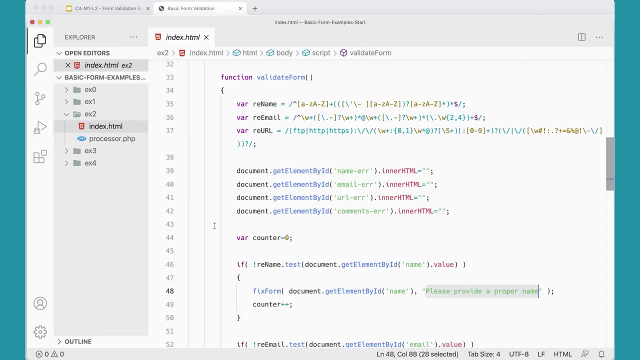 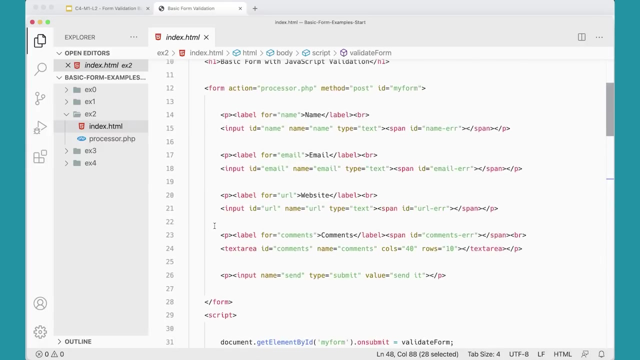 this message would still be there, even though the name is correct. So that's kind of important to understand. So, again, there's a lot going on here, And this is old school JavaScript, plain JavaScript, validation. And what's going on here is we have a form and, as you, what the key part. 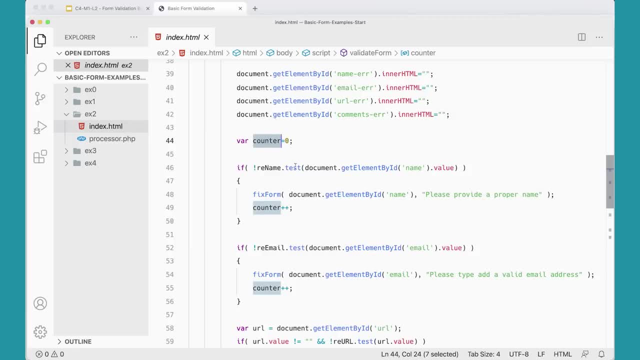 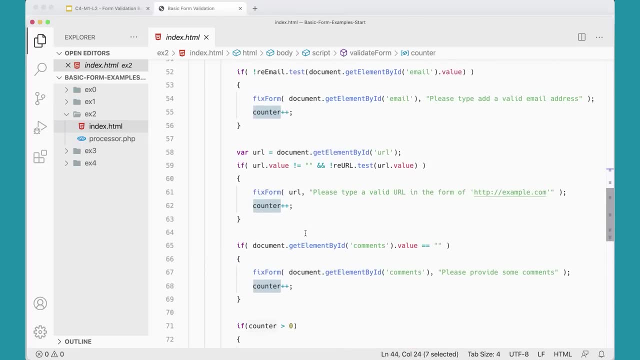 of the script is this counter here, And the counter starts at zero And, if any, you check each field and if each field does not pass, if any of them don't pass, the counter gets incremented. If the counter is ever greater than zero. 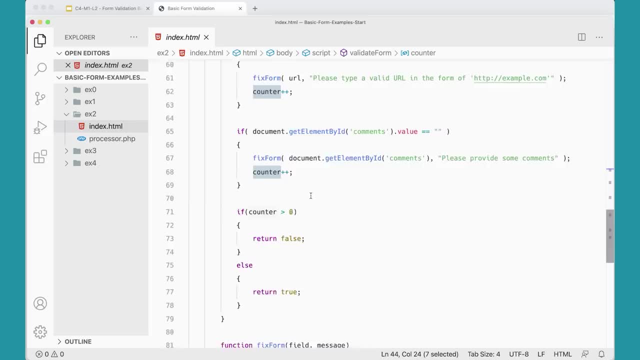 then at least one of the fields was wrong and I'm going to not process the form. Meanwhile, I'm also going to run this fixed form function that's going to put the proper message in the proper field, saying what I did wrong so I can go back and fix it. 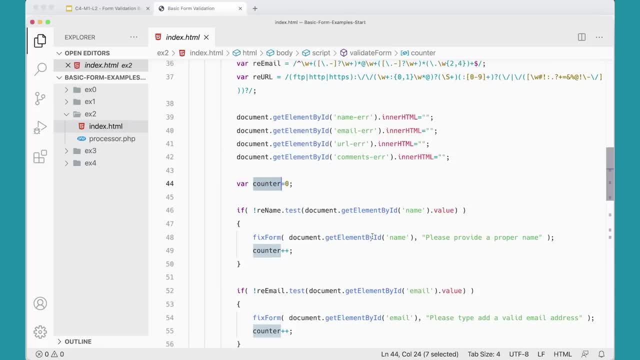 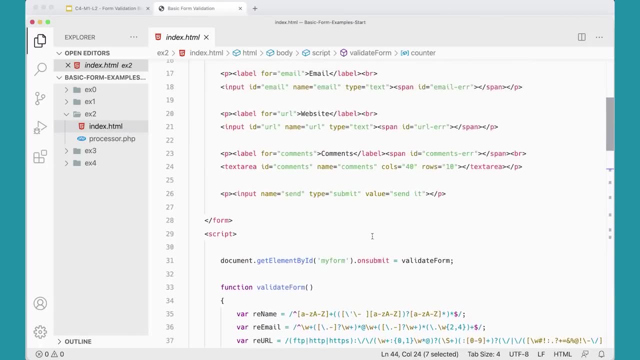 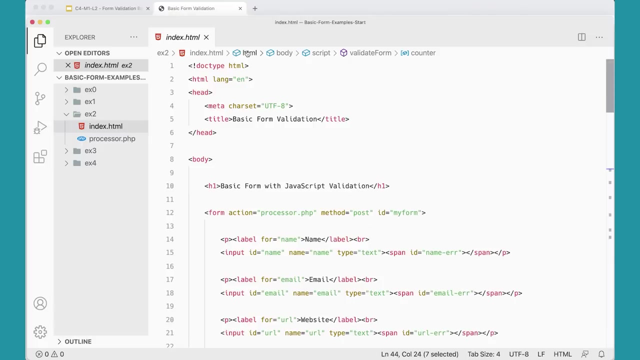 And all of that should work properly. So that gives us a JavaScript- old school JavaScript- way of validating fields, And we did form validation like this for many years. Now we've got some better ways of doing it that we'll look at in the next videos. 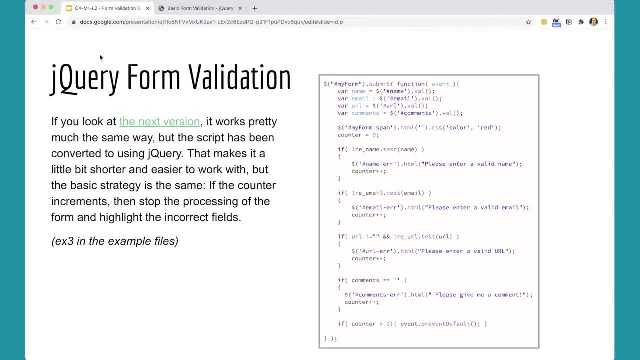 In the next version of our script we're going to use jQuery to do the same thing that we did with JavaScript And this version it's a little bit shorter, It's a little bit more compact, but it's following basically the same. 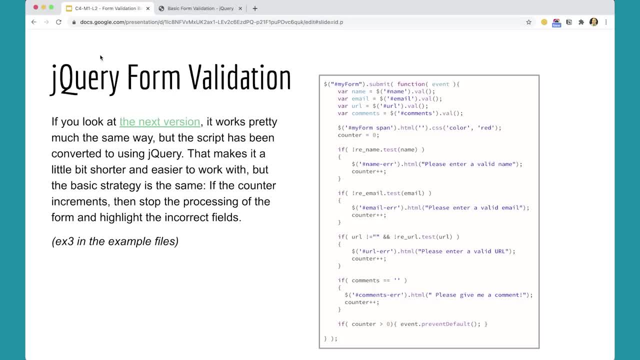 principles that the JavaScript version followed, in that we have a counter that gets incremented, and if it gets incremented, then the field is not passing validation and the entire form will not will not be validated. but it is a little bit shorter, So let's take a look at it first. 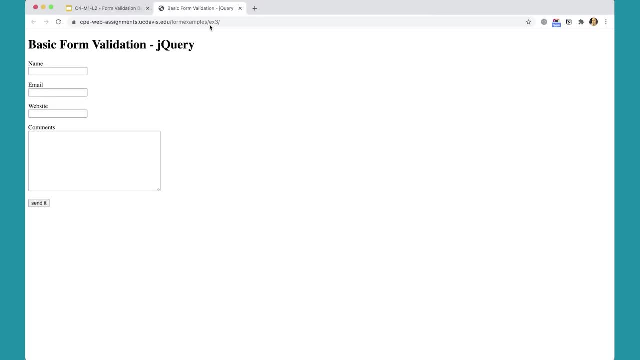 We can look at it and test it out over here And notice up here it says EX3.. So it's the same URL but EX3 at the top And I could put in. well, if I just leave the form empty and click send, we'll get some validation coming up here. 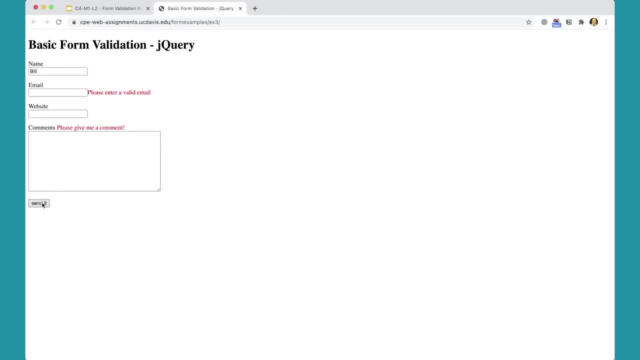 And you'll notice I can fill this. if I just fill in my first name and click send, That one goes away, but these continue. If I fill in a bad email address, you'll notice that it wants a valid email address. If I fill in a bad website. 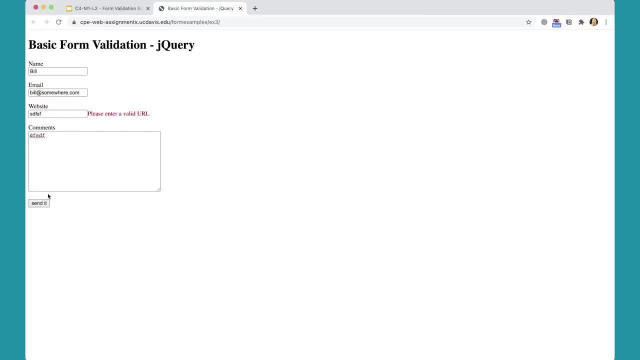 you'll notice it says: please enter your valid URL. And then we've got our message And finally, it'll go through if you fill out properly. on the back end we're using the same PHP validation in our PHP file, So we've got some back end validation going on as well. 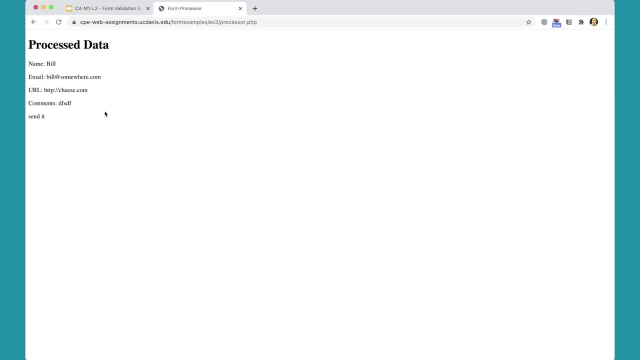 But really the front end validation should handle it. If the front end validation fails, then the back end validation will handle it. So we've got that working and that all looks very similar to what we had before. So let's take a look at the example script over here in example three. 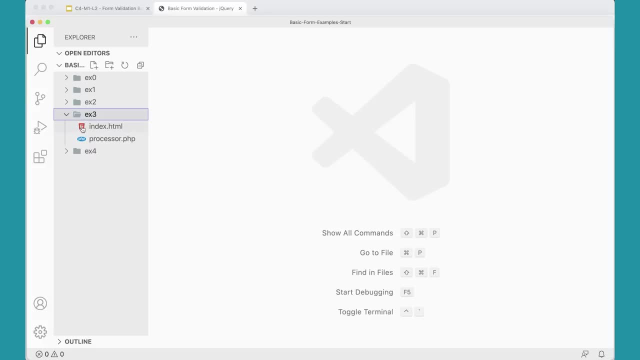 And again, I'm not having you type anything out for this script, because this is a little bit old school And I think it's just important to understand, sort of build up an understanding of where we've been with this stuff by seeing it. 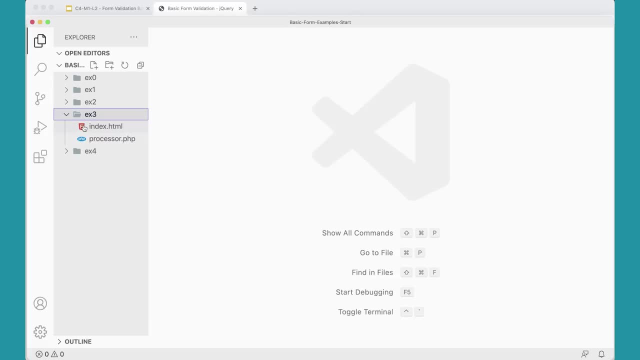 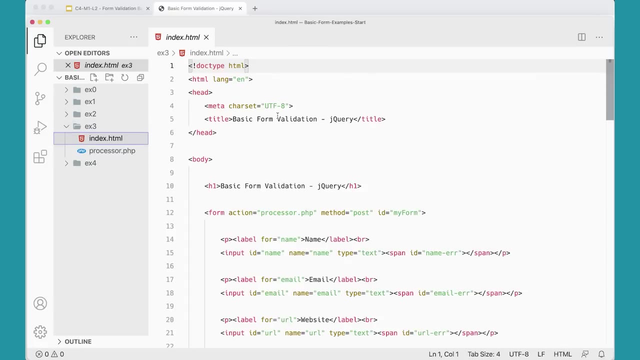 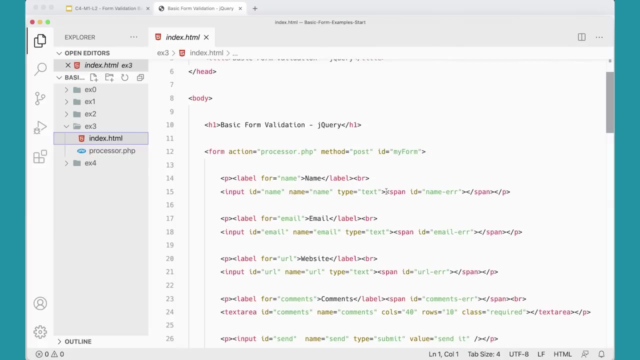 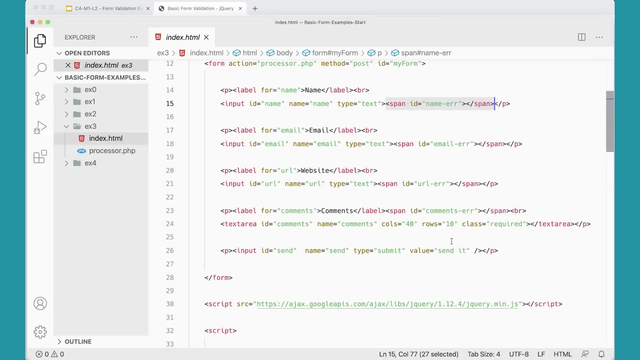 But we'll be looking at some more, some more modern ways of doing form validation next. OK, so here we are on our page, and you'll notice that the HTML is all exactly the same, with my span errors here. It's the same as what I had in the plain JavaScript version before. 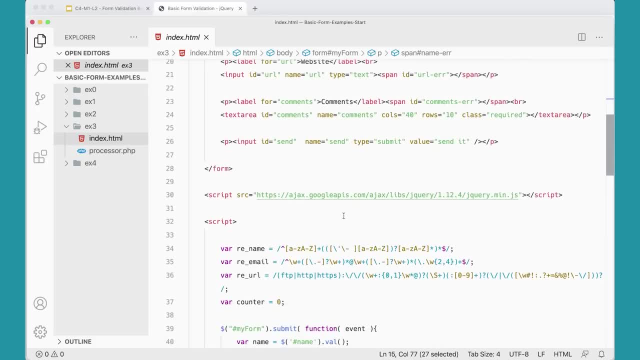 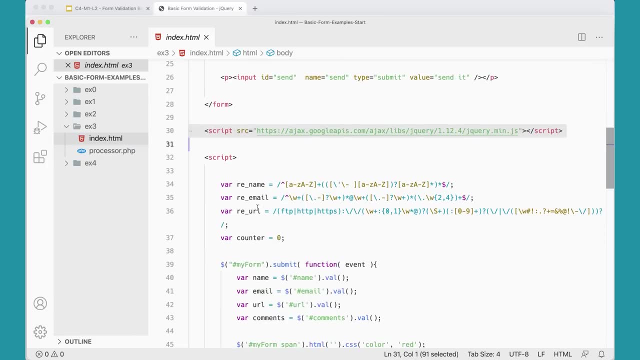 The HTML really hasn't changed. The one thing that has changed is down here. I've got jQuery plugged in. It's an older version of the jQuery library, but that's OK. And again I've got my regular expressions, so that's fine. 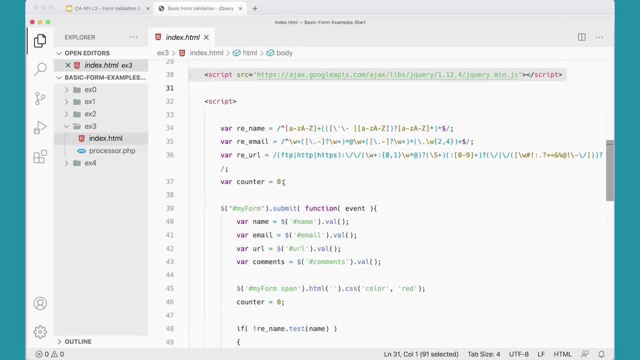 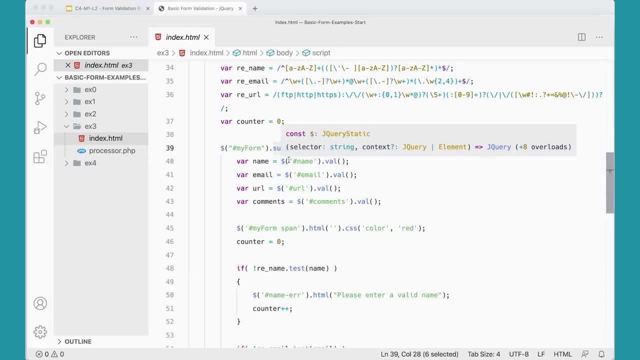 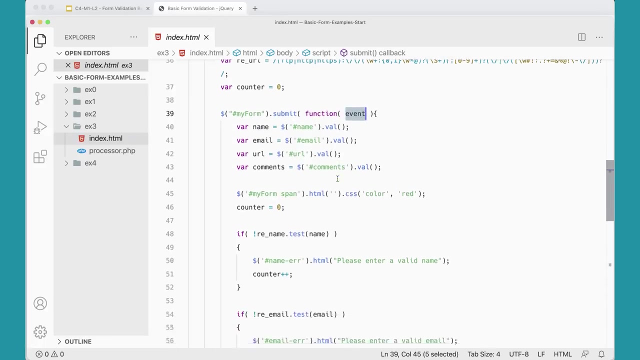 This is the same regular expressions I had before. I've got my counter set to zero And here I'm using the jQuery submit event to capture the submit of our form, and then we're running a function and passing in the event object And, just as before, I've got a counter that's set to zero. 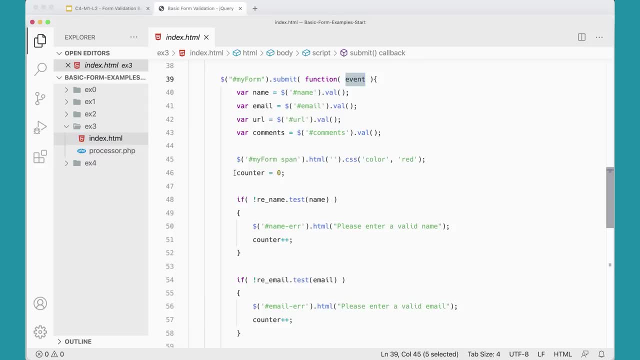 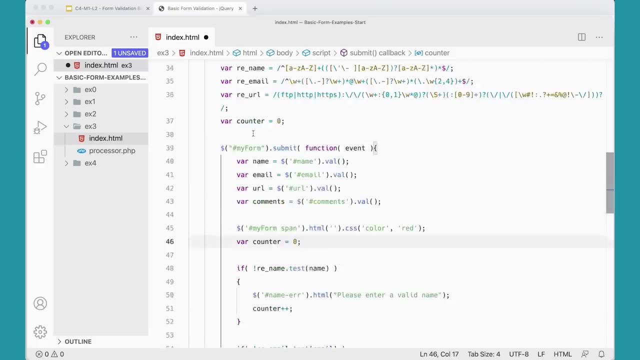 I probably should have a var in front of that. Var counter equals zero. So I've got a counter set to zero. No, I set it up there, That's why it's not far there. So I've got the counter set to zero. 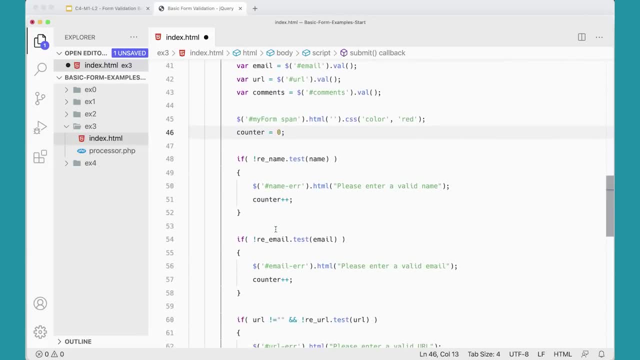 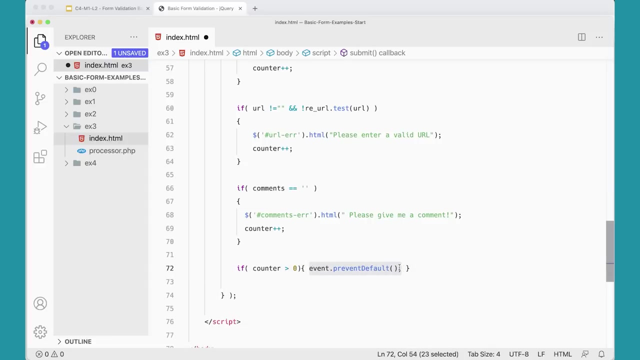 And if any of the forms do not pass, if any of the fields do not pass, the counter gets incremented. One thing that's different here is down here: If the counter is greater than zero, I'm using eventpreventDefault instead of return false. 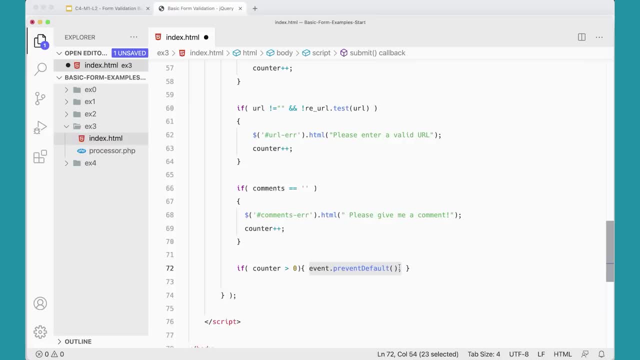 So I'm using eventpreventDefault, using that event object to prevent the default behavior of the submission of the form, and that's what keeps the form from being submitted to the PHP to be processed if the counter gets incremented. If it doesn't, then it gets submitted, just fine. 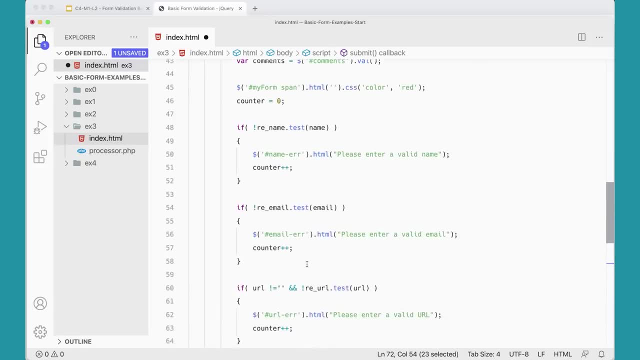 If it doesn't get sent in. another thing that's different is I don't have a separate function for fixing the fields Here. I'm just using a little bit of jQuery to say: go get that field name-err, change its HTML. please add a valid name. 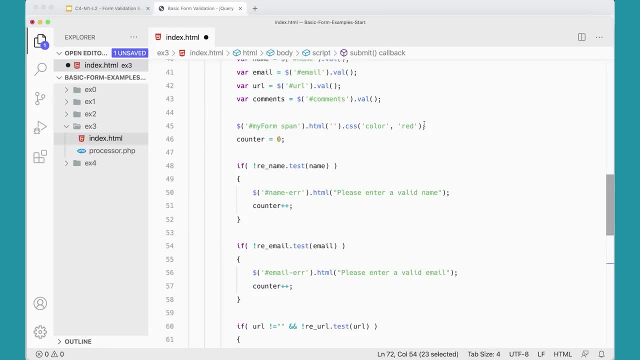 And up here I've got this little thing here that will turn that red automatically. So that's all fine Up here. these variables here again are just getting those fields, getting the values out of those fields, so that that should all just work. 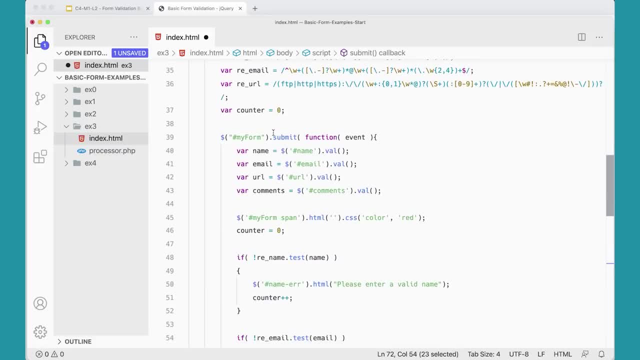 And get kind of set up. So it's a much simpler version of the exact same thing that we did with the plain old-school JavaScript. Here, these forms are getting emptied out each time. So because jQuery can work on a group of objects, I don't have to set each one. 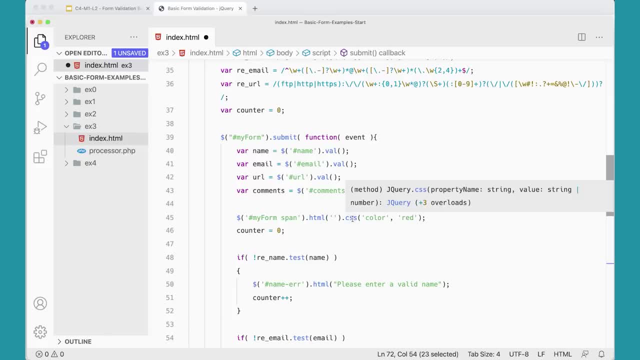 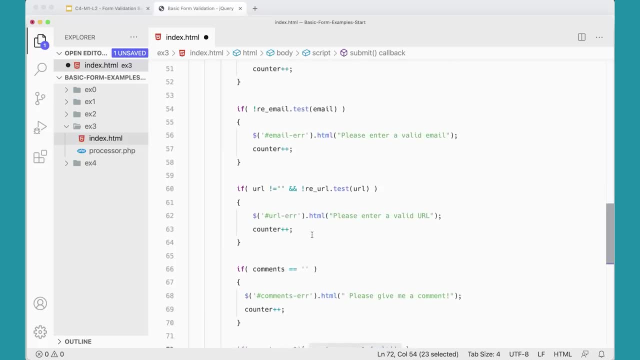 of them separately. I can just set the HTML and all of these to empty. Let's set the CSS to color and red for them, So that kind of works sort of nicely there. So it's kind of a nice simple version of the script that we did. 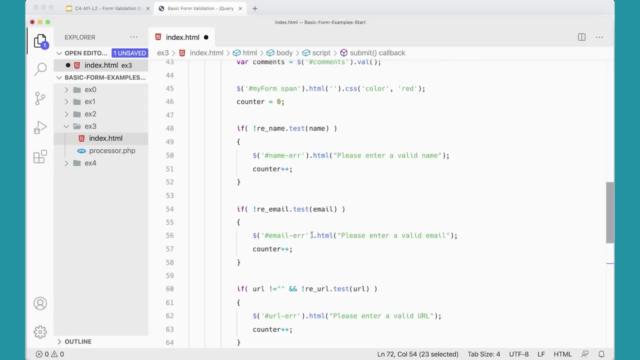 It's still a little bit cumbersome. If you had a longer form, you would have to do this for each and every field on the form. So imagine a long form. You would have a lot of JavaScript here or jQuery here to do that. 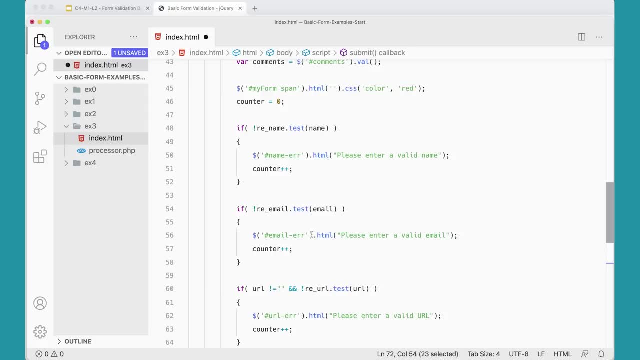 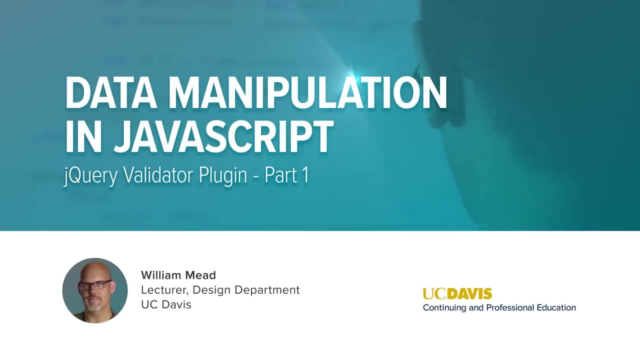 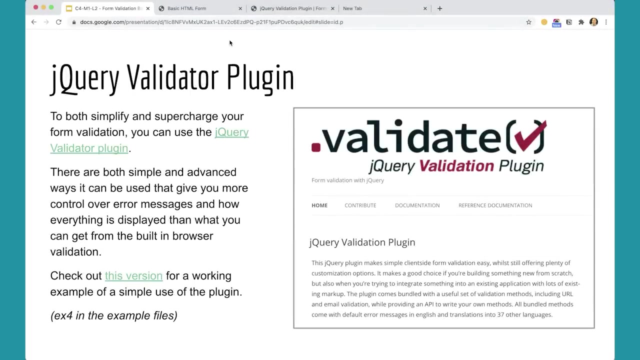 And it works. But again, this is kind of an old-school method for doing this. The next version of our script is going to use a jQuery plugin, the jQuery Validate plugin, which is a fantastic plugin for doing form validation. It provides both simple and advanced ways. 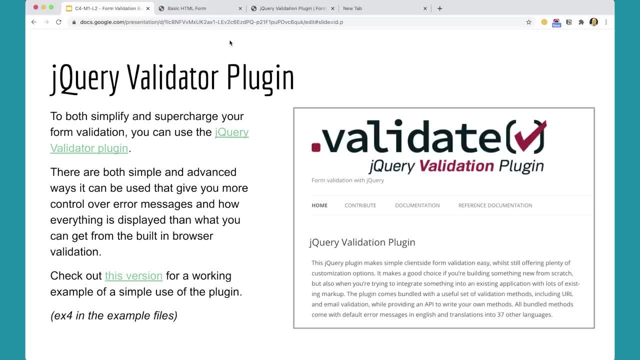 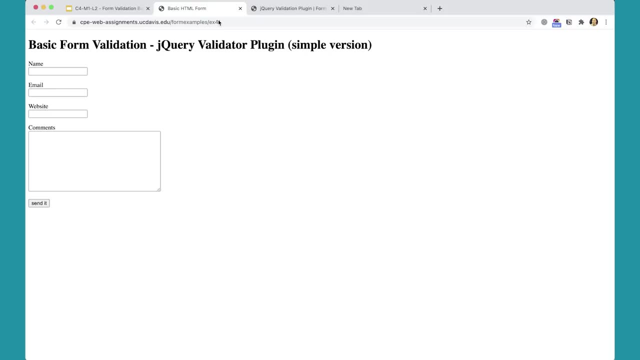 of doing jQuery validation, and the documentation is spectacular. It's one of the oldest jQuery plugins out there and it's a really great one to use for validating forms. To give it a try, you can go to the same website, but ex4 over here is the folder name instead. 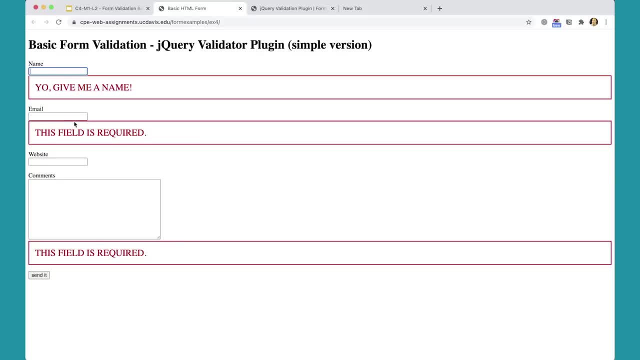 And if I just click send it here, you'll see. Yo, give me a name. You can see I've styled this stuff a little bit, Not very nice, but it's here. And then, as I type in my name, notice that error goes away right away. 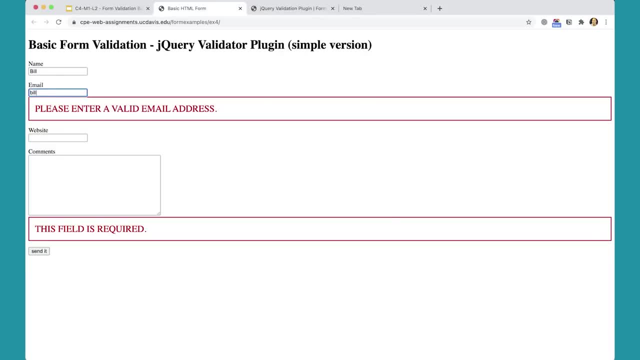 For email. if I type in an email, it'll immediately switch to please enter a valid email address Somewhere dot com, like that. If I type in a website, if I type in a bad website and click send, it'll say: enter a valid URL. 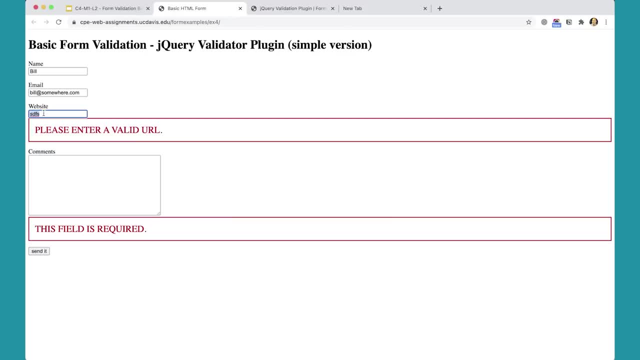 If I type in something. well, we already saw. So we just need to do HTTP colon slash, slash some site dot com, And then I can type my comments, hello and send it, and then it will finally go through to the same PHP file that we've been using since we added our PHP validation. 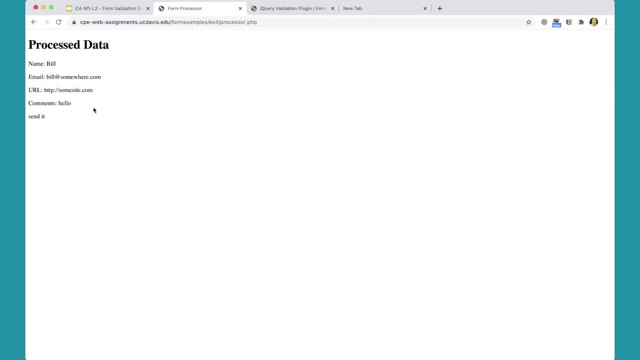 in the second version of our script, or an example one back there. OK, so that's going through and working, So that's great. So in this version you're finally going to get to type a little code and you'll see why we didn't type all that code from the previous versions. 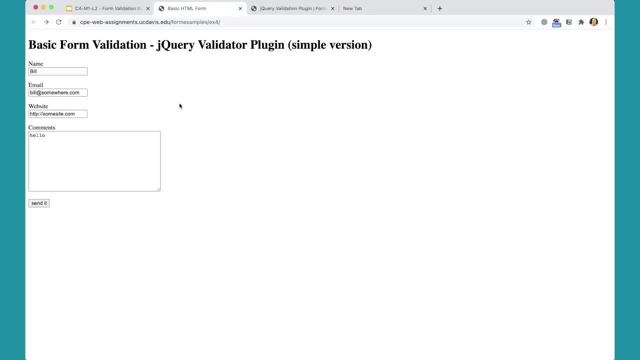 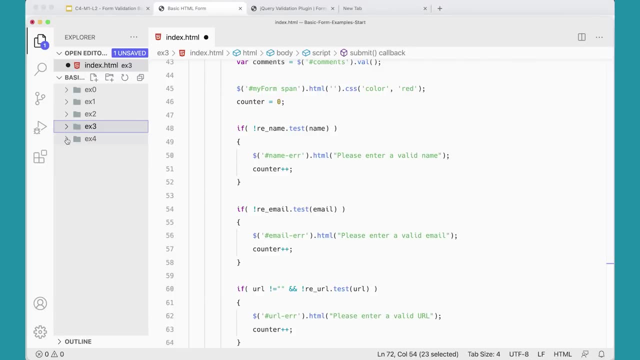 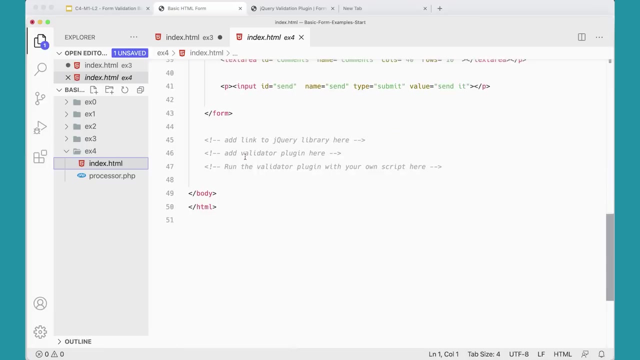 because this one is so much easier to use. So the first thing we need to do in order to make this work- if you go over to the example files and we go down to example four here, the first thing we need to do to make this work is we need to add the jQuery library here. 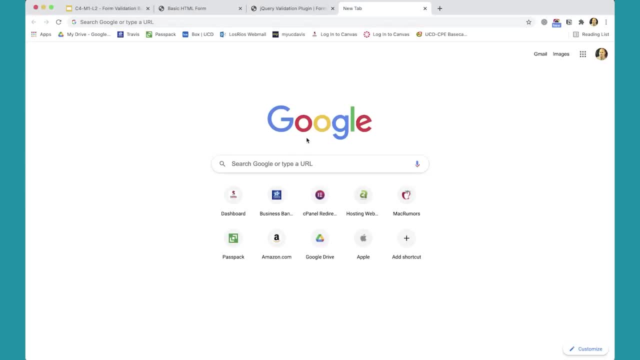 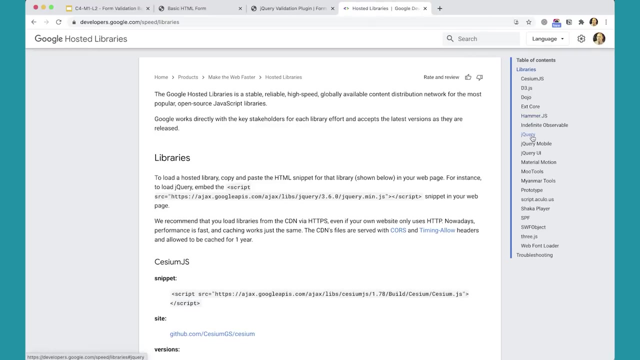 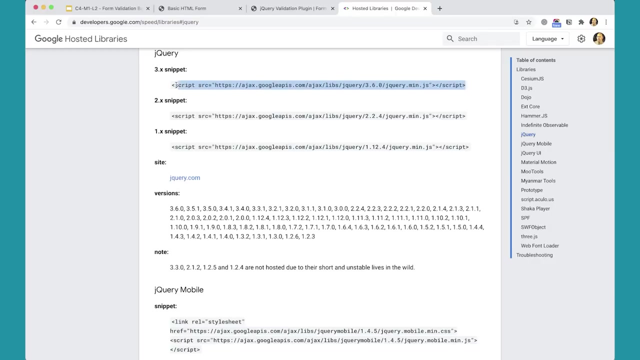 So I'm going to come over to a new tab over here. I'm just going to Google jQuery, CDN, Google, something like that- And I go to the hosted libraries for Google developers and go down to jQuery over here and just grab this snippet right here for the latest version of jQuery. 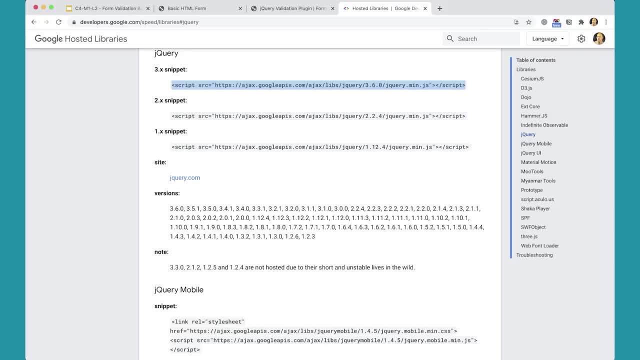 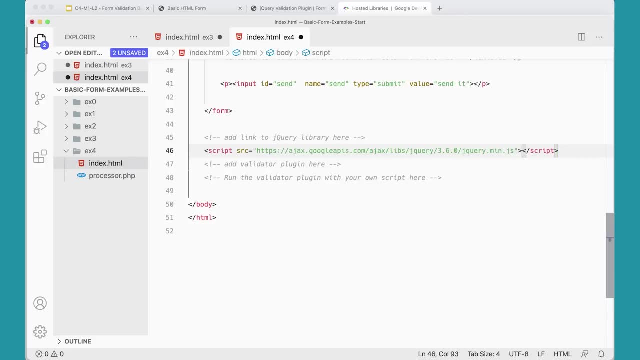 So I'm just going to copy that and paste it here: Add link to jQuery library and stick that there. Great Down here I'm going to add a link for another script: SRC equals, quote, quote. And what am I going to put in here? 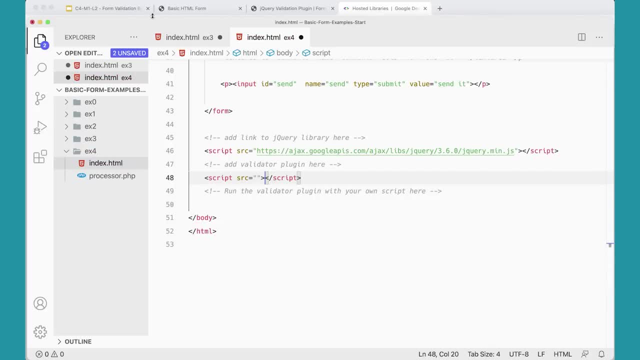 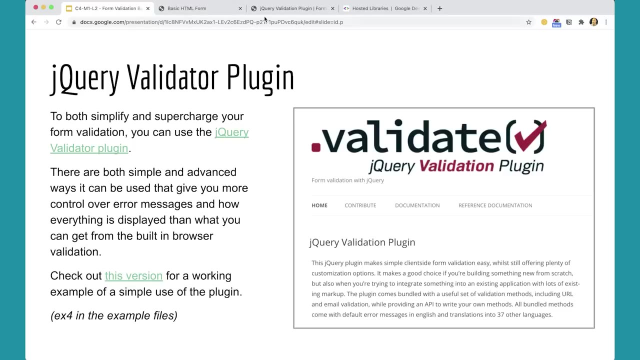 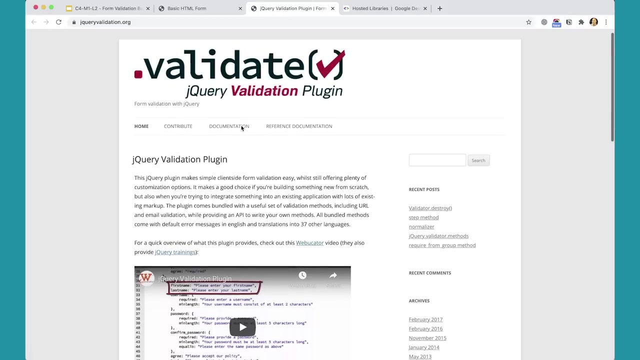 I'm going to put my validator plug in. So if we go over to our slides here and you can click this link, or I will provide a link with the lesson that will take you over, Or you can just Google jQuery validation plug in and it will take you to this website here. 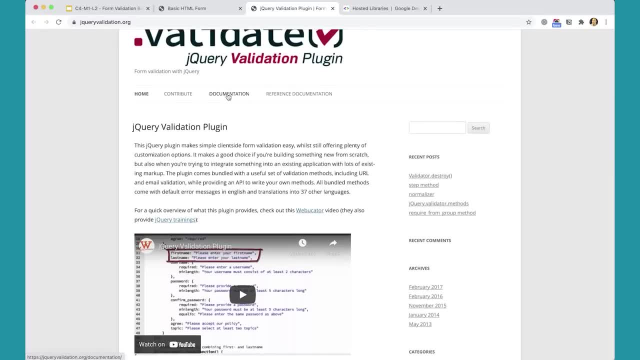 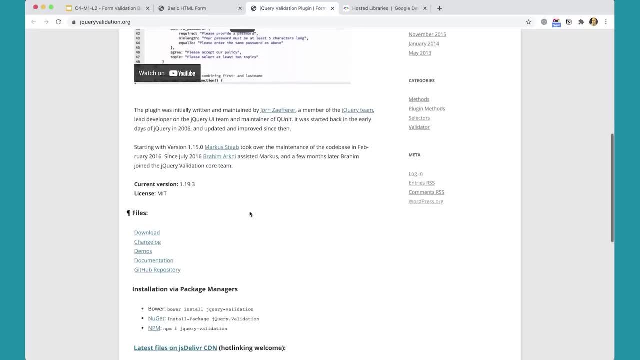 And this website has great documentation About how you can use the plug in. It's got all kinds of good stuff on here, along with video, And we're just going to do kind of a very basic version of the use of this plug in. 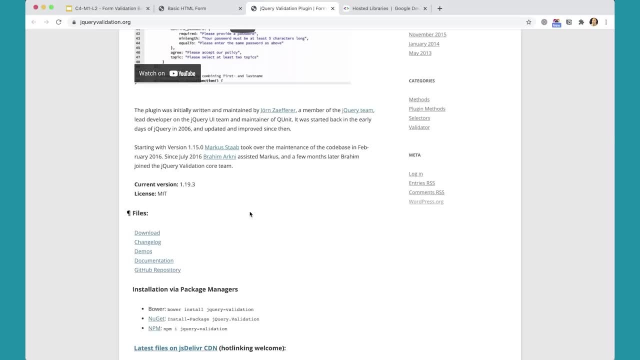 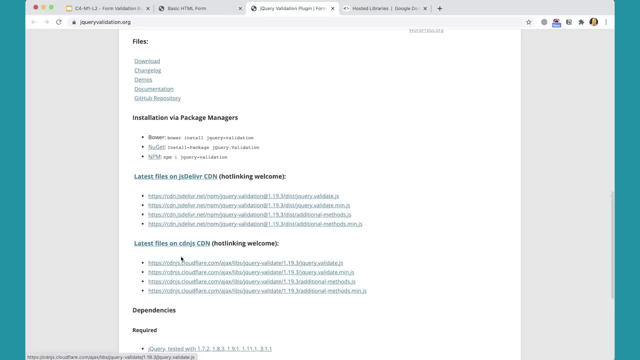 Just so you can kind of see how that works, for right now They give you some different ways of linking to it, And here we've got the CDN, JS, CDN- That's the one that I like to use And notice. we've got validatejs, validateminjs. 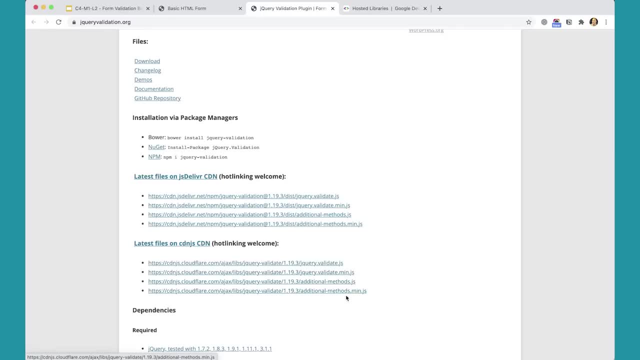 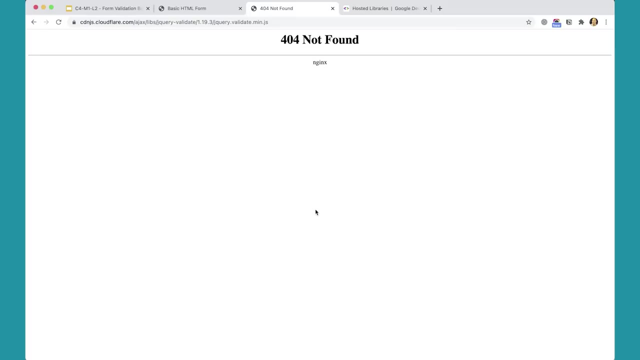 And then we've got. we've got some additional methods and an additional methods, And you would have to read about these in the, in the documentation. But really what we want is the minified version. Whoops, Not sure why that's not coming up. 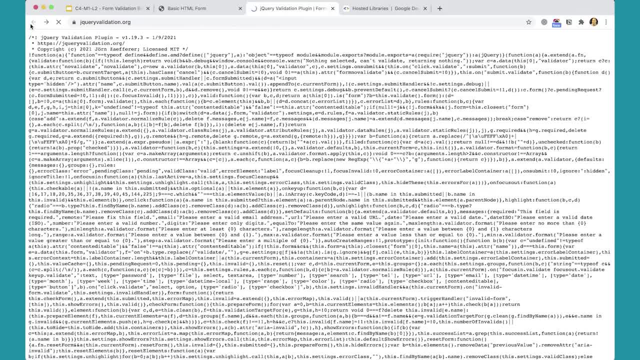 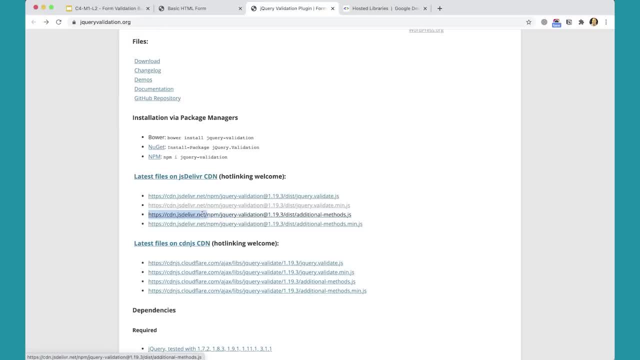 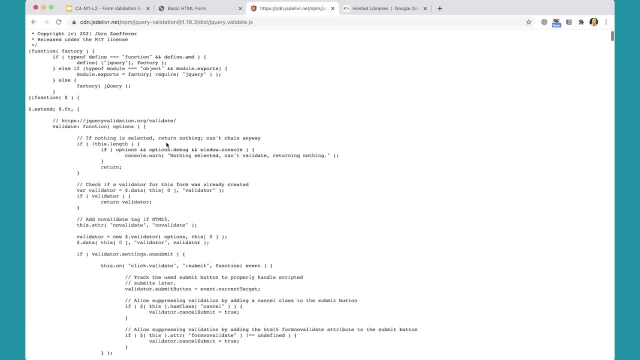 There we go. I guess we'll use this one. We want the minified version here, So I'm just going to copy that URL right there And again, the minified version will be smaller. If you click on this one, you'll get sort of the expanded version. 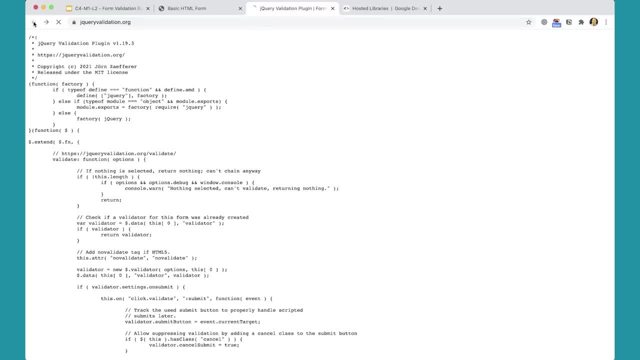 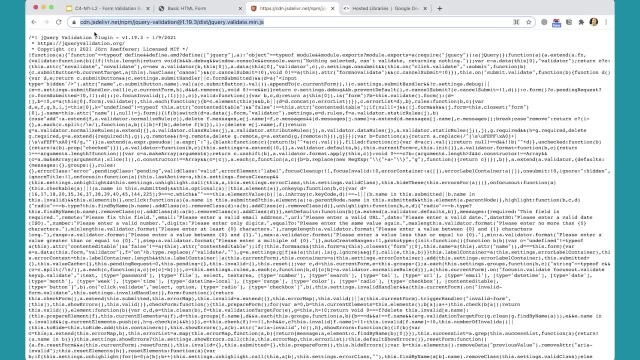 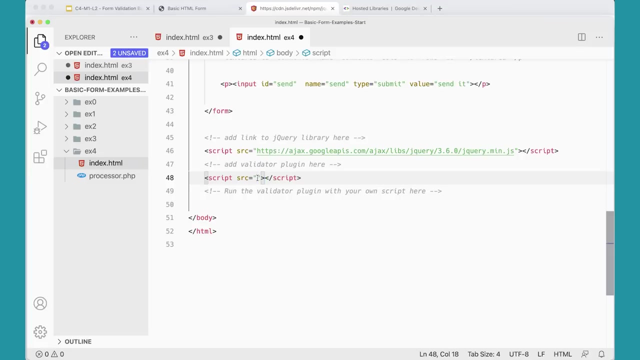 But that's going to be a larger download. The minified version has had all the white space removed, So that's really what we want. right, there is that minified version, So I'm going to copy that version and then come over here and stick it inside my source attribute here. 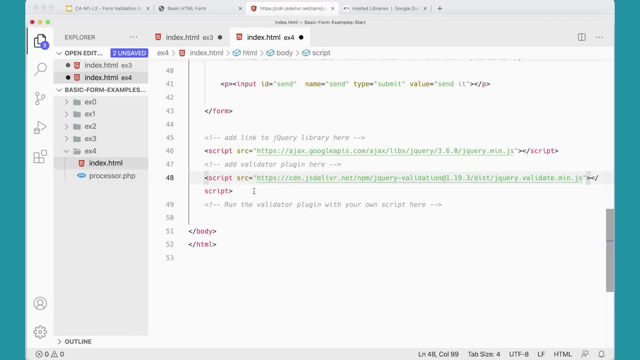 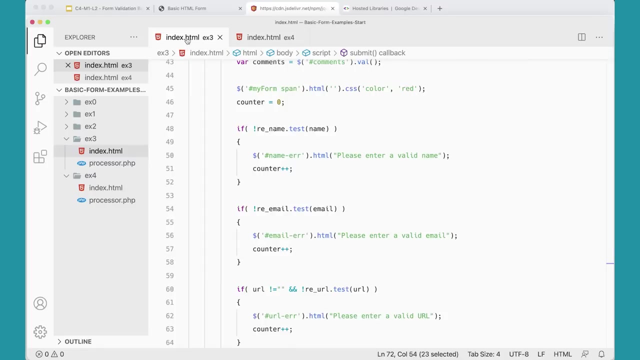 OK, So now we've we've linked to the jQuery validator plugin And then down here we need to run our own script and save this file. Sample three: done with that one, I'm going to close my explorer because that's kind of long and sticking out there. 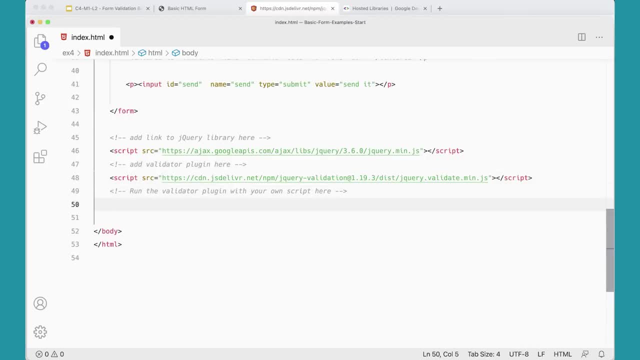 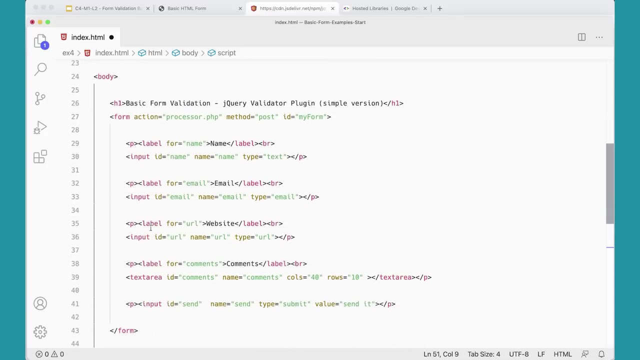 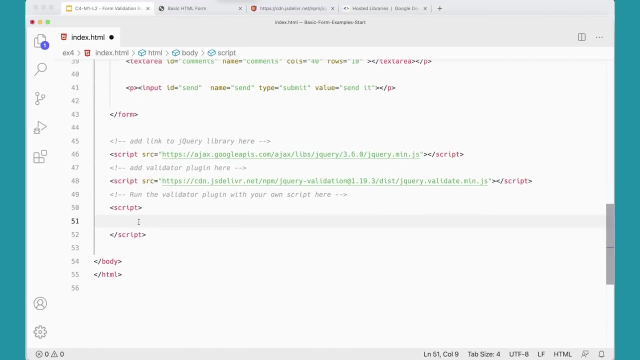 But here I'm going to run my own script And this could go on to an external file, but it's really simple. All I need to do is get my, get my ID for my form and tell it to validate. Start, of course, with our jQuery object. 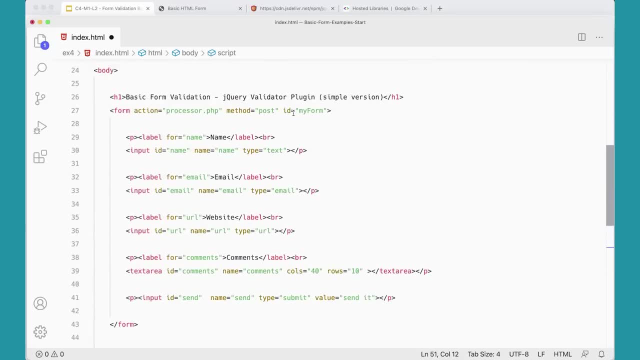 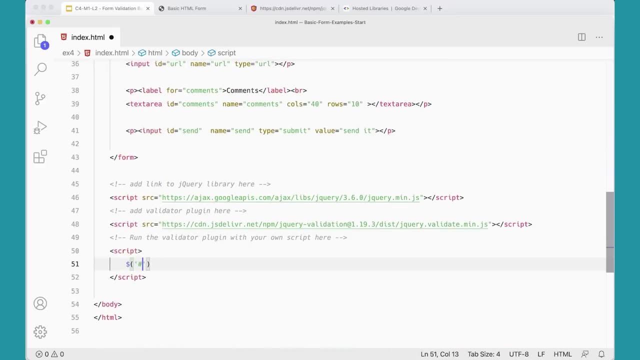 And what am I getting? I'm getting my form, this ID for the form itself, And my form Dot validate. My spacing got screwed up there. All right, dot validate. This validate method is a method that's provided because we have the validation. 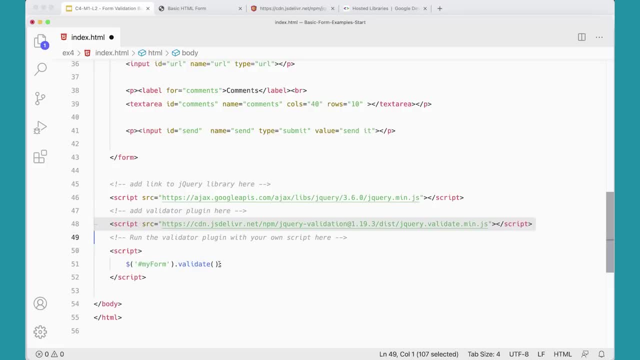 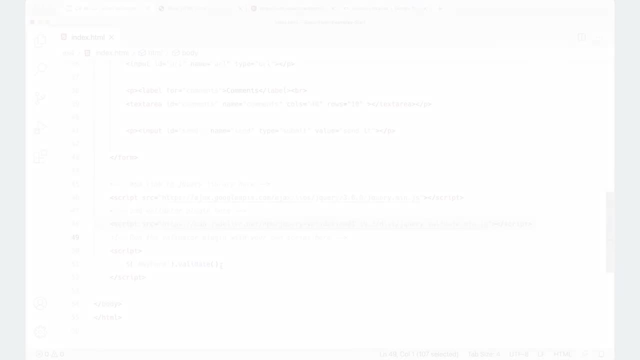 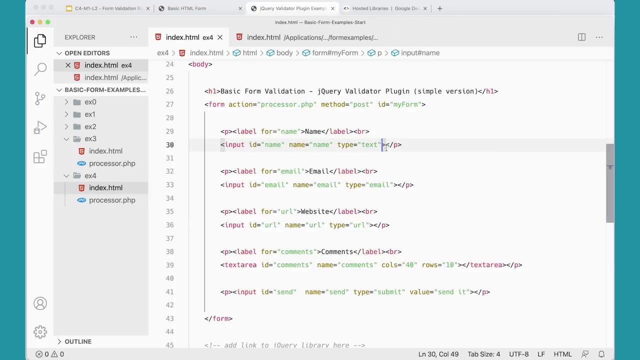 plug in. This is not a native part of jQuery, It's part of the plugin. Because we have the plugin we can use validate. Let's see what happens Before we can test this. we just need to require some fields. So come up to the input here and add. 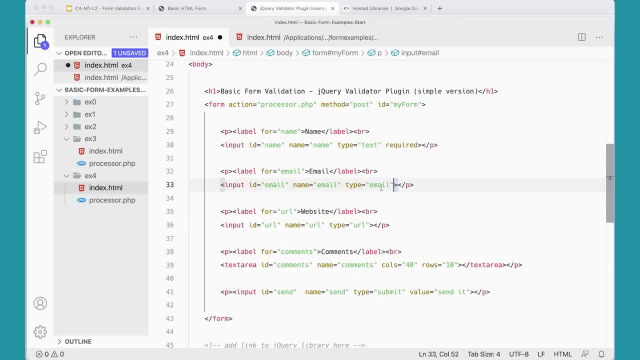 required in here, Also on the email one, And we're going to skip the URL, but you'll see that it will test the URL And also in the text area, Add it there. Make sure you add it before that angle bracket, before the closing text area tag. 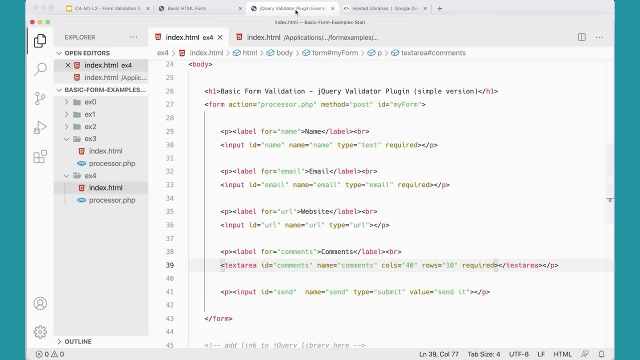 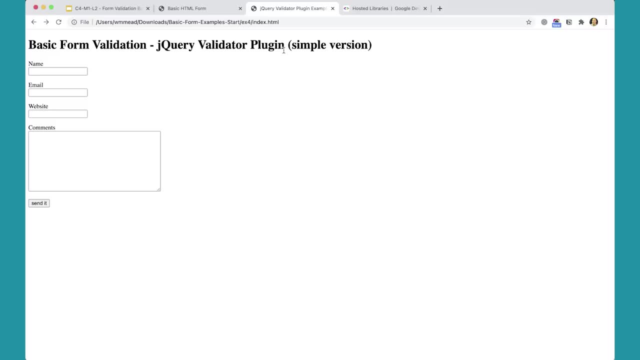 OK, so I save that and then I'm going to come back over to my form and I'm just loading this locally. the PHP is not going to work properly, So if it goes through to the PHP, we'll actually see the PHP on the page. 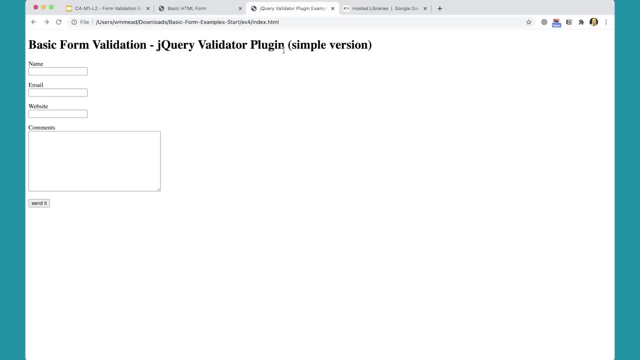 But we don't really care about that. We know that our server side validation is working, So that's OK. We can just run this locally off here. Alternatively, you could run it through MAMP or XAMPP or WAMP or one of those. 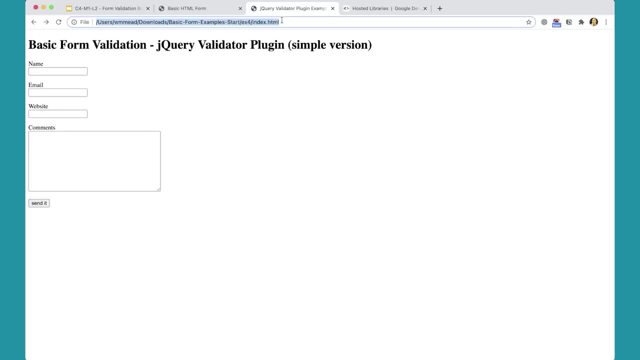 local servers or put it up on a web server somewhere, And it will work exactly the same way that this one up on the web server here works. So yeah, so, but for now this should work just fine. So I'm just going to refresh this page. 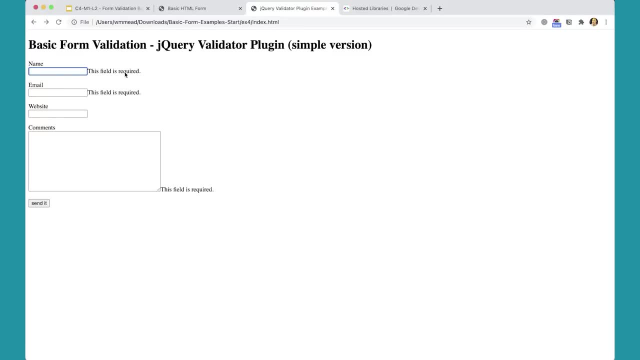 And if I just click send it, you'll see we're getting. this field is required. This field is required. This field is required And if I type something in here, that message will go away down here. If I start typing an email address, you'll notice that it will switch to please. 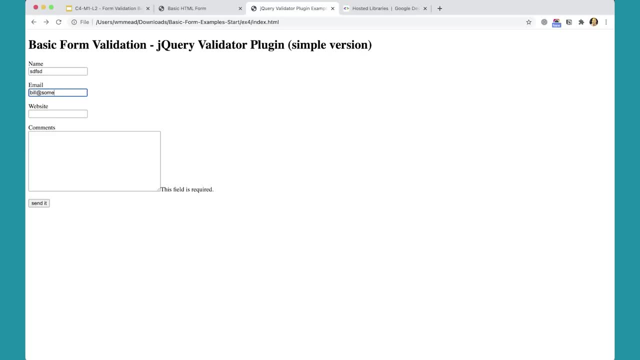 enter a valid email address at somewhere, dot com, and then website. If I put in a bad website, you'll notice it will pick that up. Please enter a valid URL. As soon as I clicked into this next field, it picked that up. 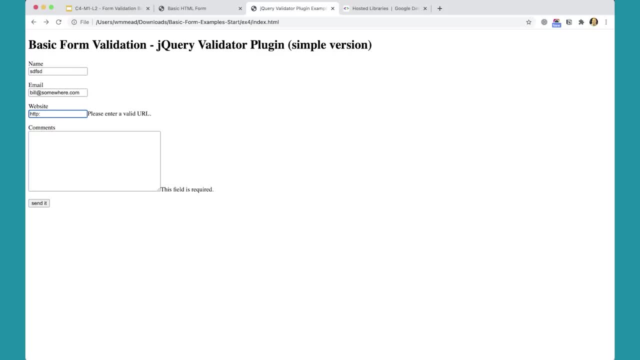 even though I didn't say that that field is required because it's set as type URL. the validator is picking it up. slash some site dot com, I don't know something like that. Hello, And then if I click send it, I get my PHP. 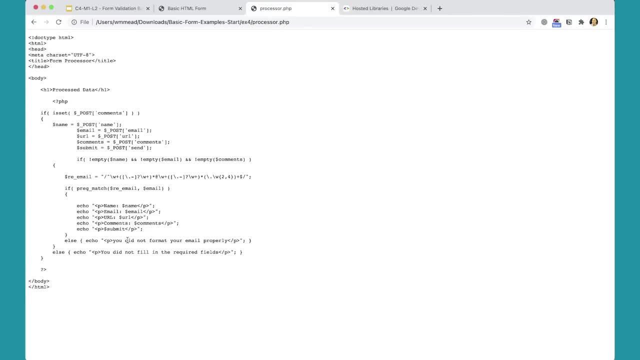 which is not really what I want. I'd rather get the return file, but I'm just running it locally off my desktop, So the browser doesn't know what to make of all this PHP, So it just shows it to me. OK, but the validation is actually working. 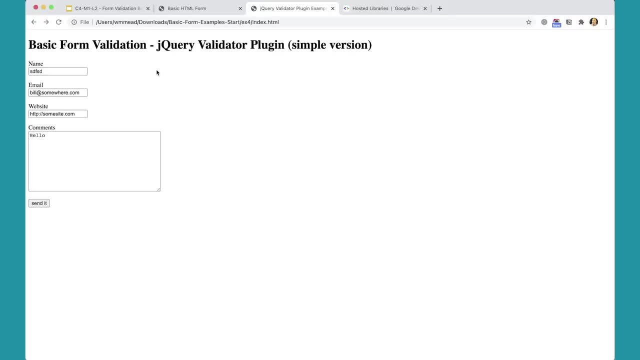 I can take this even further by adding some additional titles in there. So if I wanted to adjust the names of the fields that show up, we can do that too. Also, you'll notice that if there's an error, It creates a, it creates an element here. 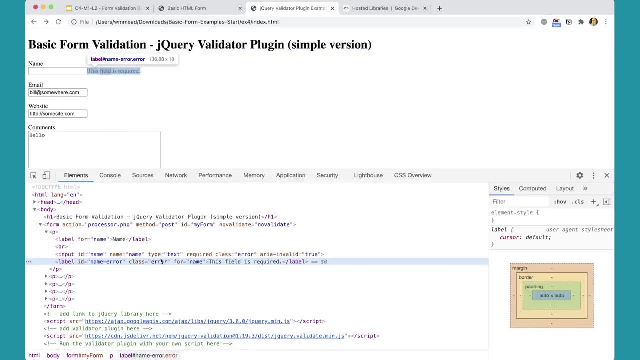 that I can see. that has the name dash, you know, as class error on it here on this label field is required. so it's creating a label here And giving also a class of error on this input here as well. So you could hook into these classes to do. 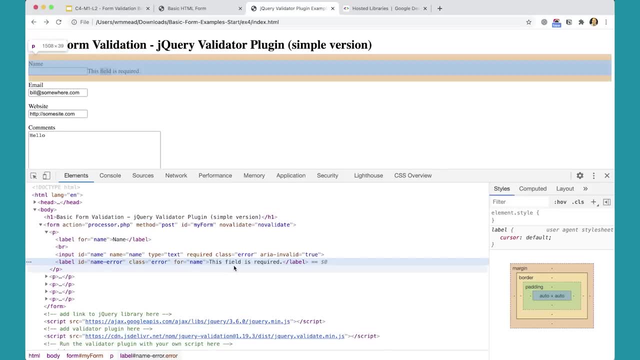 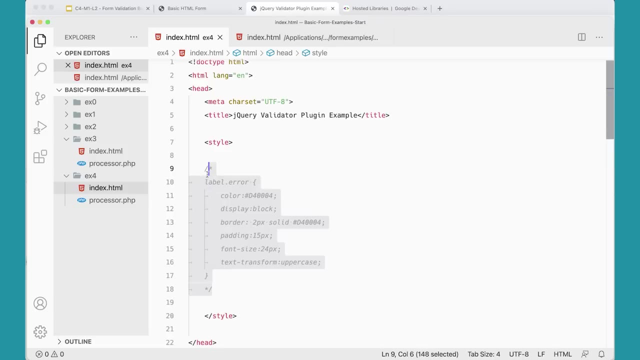 something with this stuff if you wanted to, which is pretty nifty. So I could come back to my page here and add: I could uncomment out this Style that I have here And now, so you could style these errors any way you want, which is pretty handy. 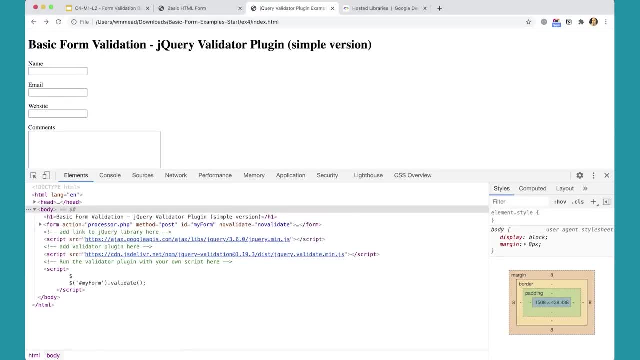 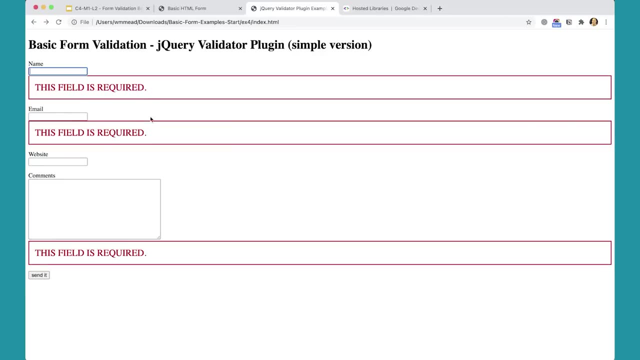 So now, if I come back and refresh this and try to submit it, you'll notice that it will take on that styling, which isn't very nice, But but you could do whatever you wanted with styling for this, which is which is really pretty cool. 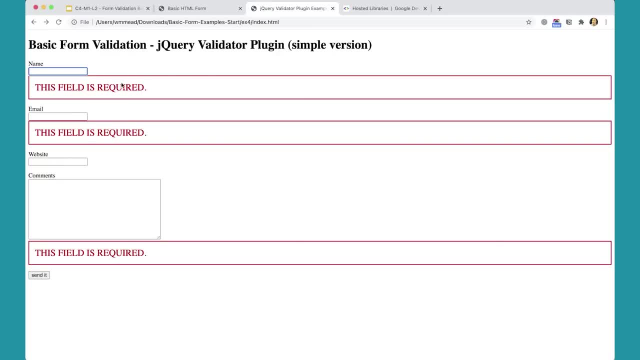 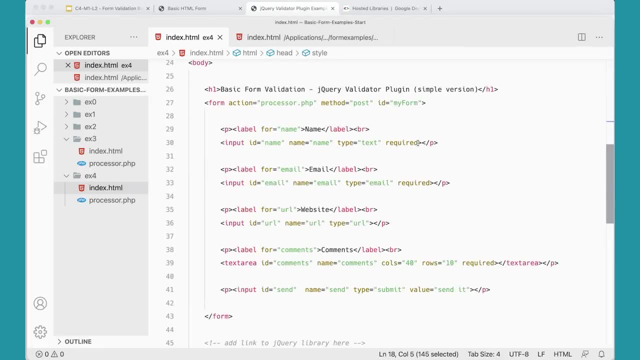 You can do that. And finally, if I don't like these labels in here, you can adjust them a little bit by adding a Title in here. Title attribute, title equals: Yo, Give me a name. I mean, it'd be better if you put in a nicer, more gentler title than that. 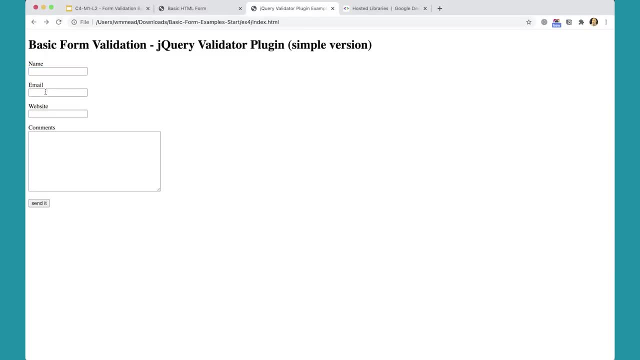 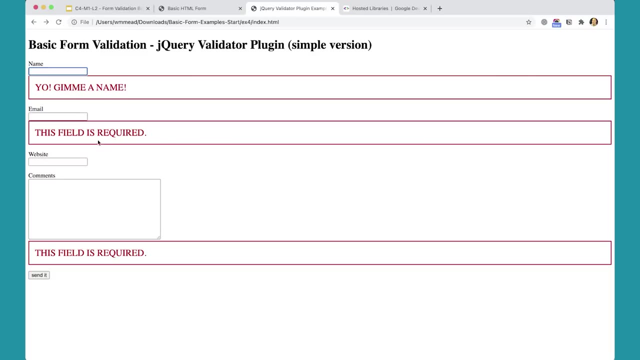 but that'll work. So now, if I don't put that in there, you'll notice that it uses that instead of the default text for the field, which is pretty nifty as well. So there's a lot you can do with the jQuery. 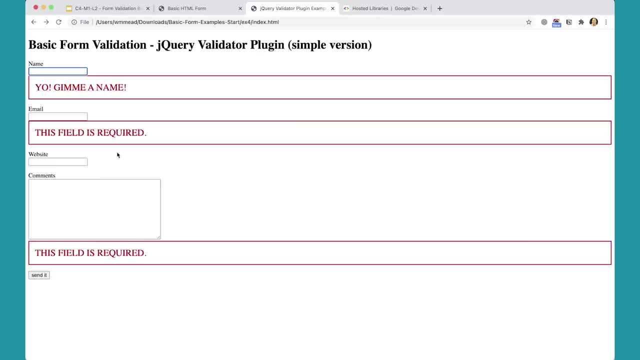 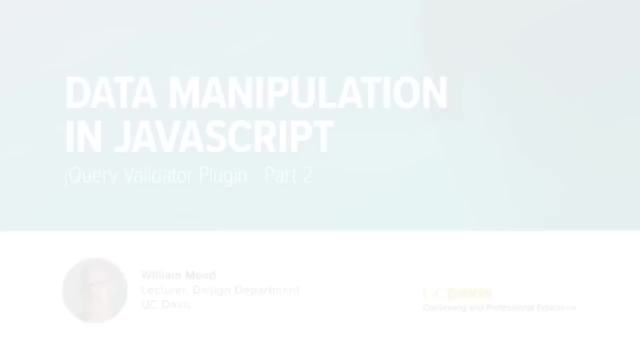 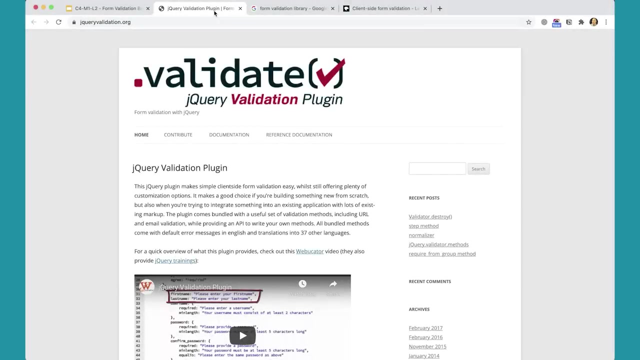 validator. and this is just the simple version. in the next lesson We'll look at some more complex features of the jQuery validator plugin and we can get into a lot more with it. But before we move on from this lesson, Before we move on from this lesson, 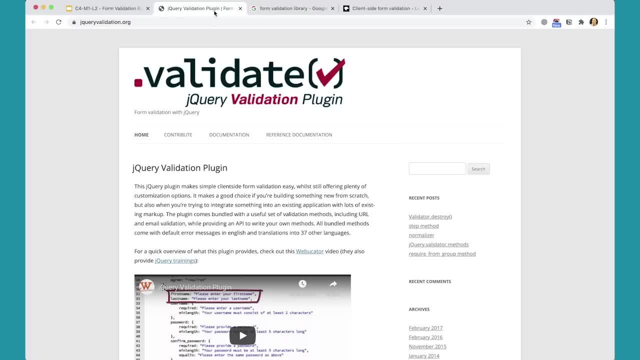 I want to talk a little bit more about form validation, and this jQuery validation plugin is really fantastic. It's got a lot of really great features, and we're going to look at some of the more advanced features in the next lesson. However, if you're over jQuery and you're ready to look at something else, 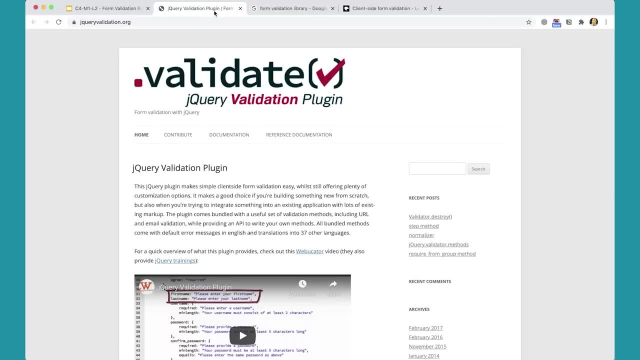 other than jQuery. there are other libraries out there that are designed specifically to do form validation. So if you don't want to load jQuery and have all the overhead of having to load the jQuery library entirely, you can look at plugins or not plugins. 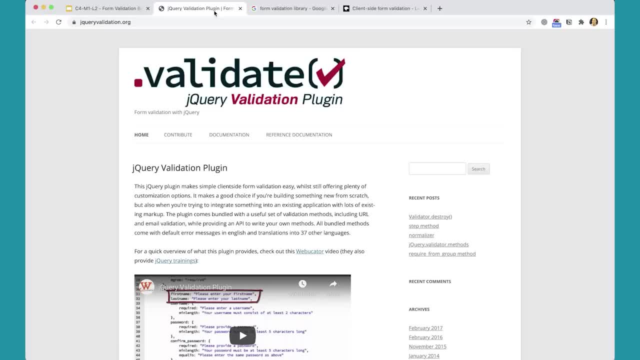 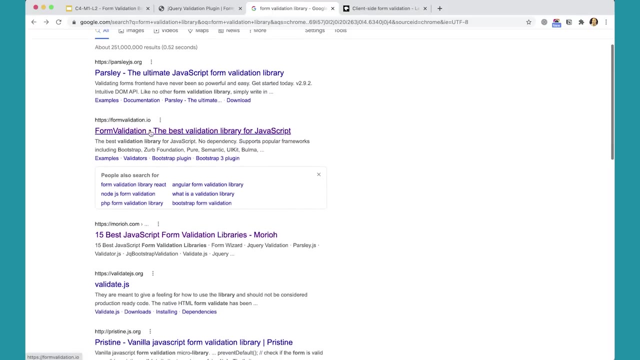 but libraries that are specifically designed to do form validation without anything else, and that could be a more efficient way of doing this. And if you just Google form validation library, you'll get a whole bunch of stuff, including this form valid. They're claiming to be the best- zero dependencies and explore features. 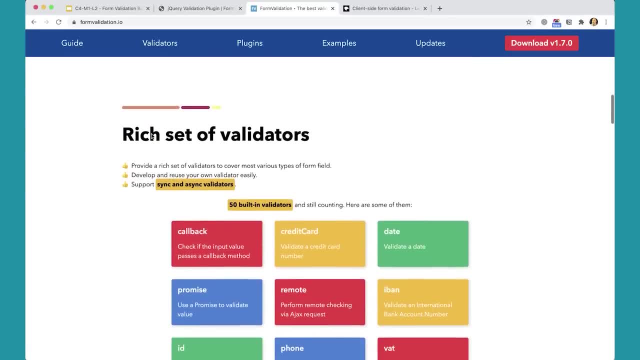 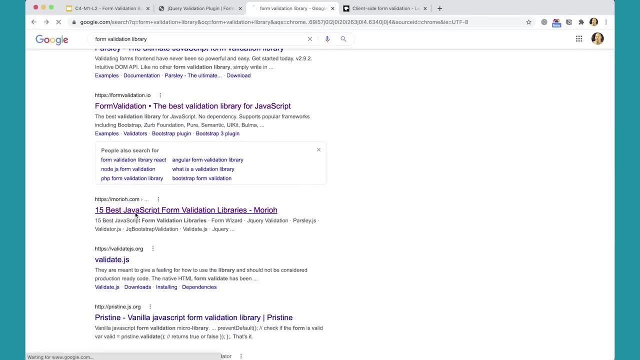 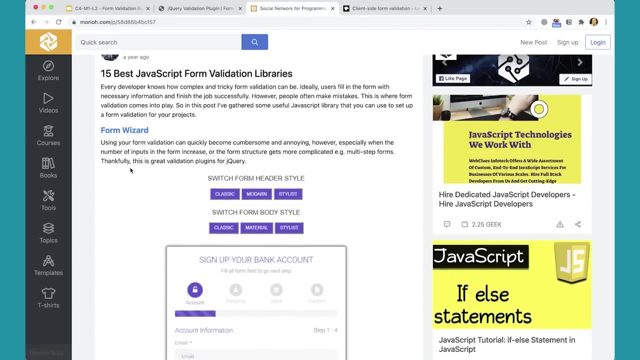 And you know you don't need any jQuery to do this and you can download it and use it, And that's great. I've never used that one. Or there's this link here that will take you to 15 best JavaScript form validation libraries: form wizard. 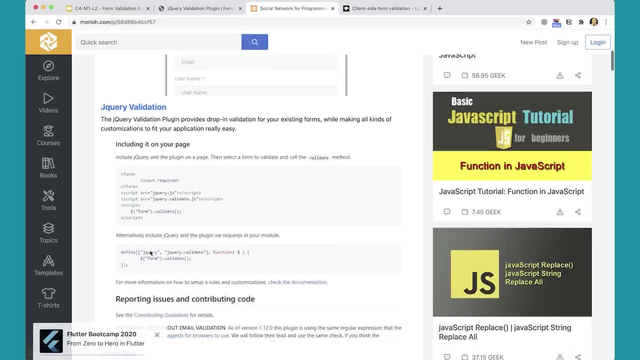 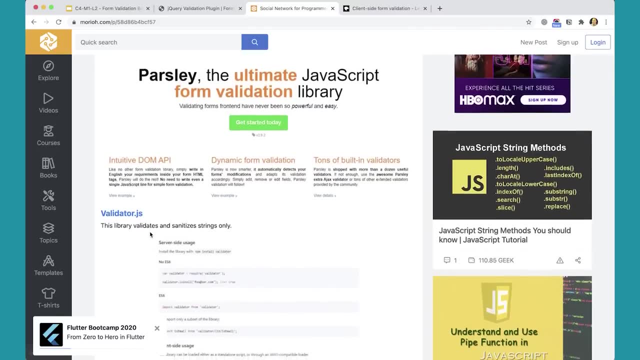 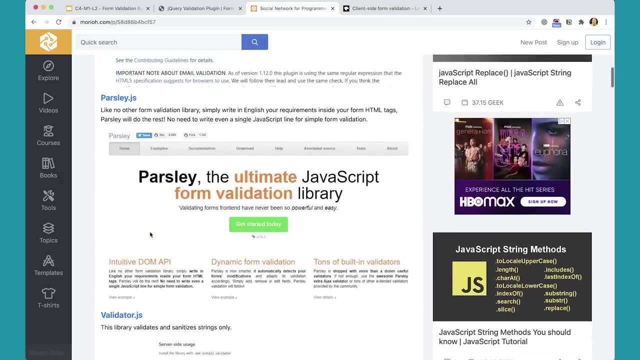 jQuery validation libraries. That's the one that we've been looking at: Parsleyjs, Validatorjs- I've looked at this one before and it works really nicely, So there are a bunch of different options out there that you could use for form validation without having to download. 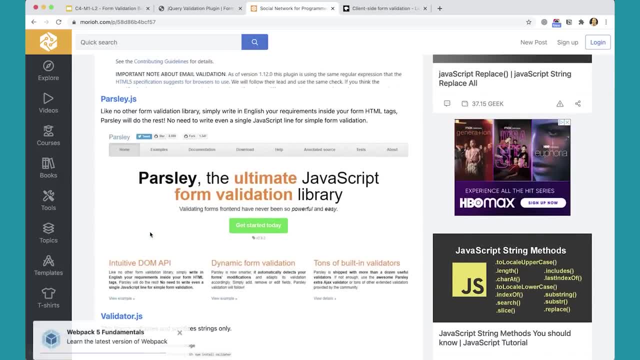 the entire jQuery library. So if you're not using jQuery for something else on your website, maybe not have it get installed just to do form validation, because you could probably find something that's going to be more lightweight that will help you do form validation more efficiently than downloading all of jQuery as well as the jQuery validator plugin. 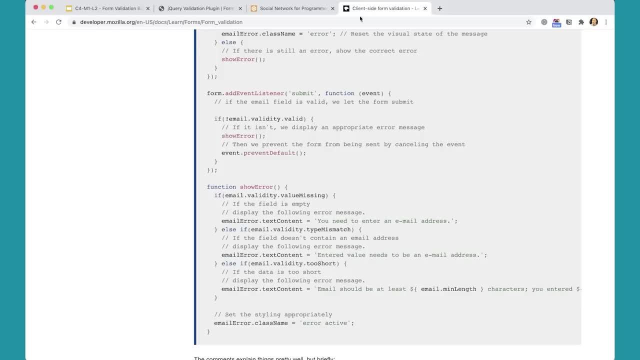 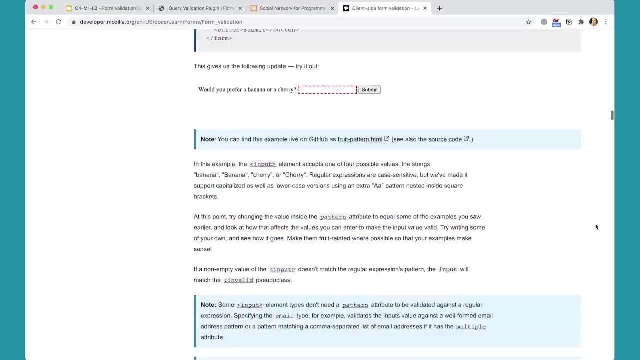 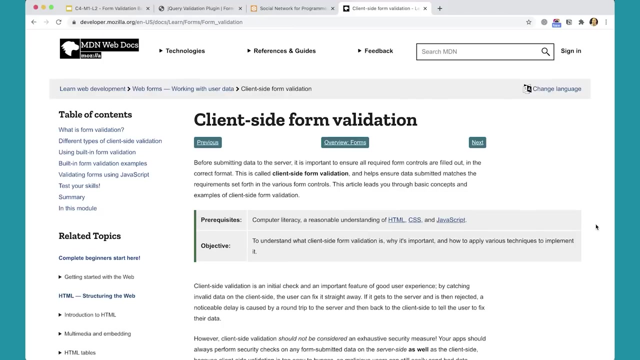 So there's that. The next thing I want to mention is that there's a really great tutorial on the MDN website here that is- and I'll leave the link for this in the lesson as well- And this is all about client side form validation. 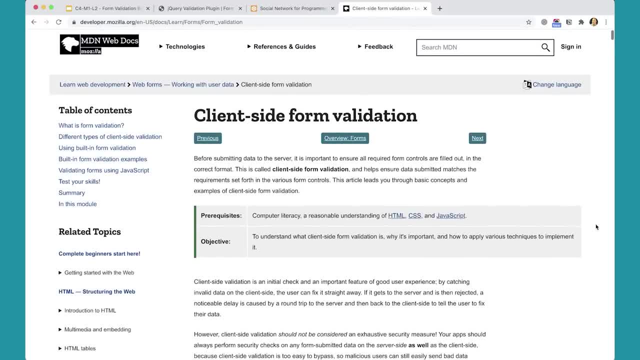 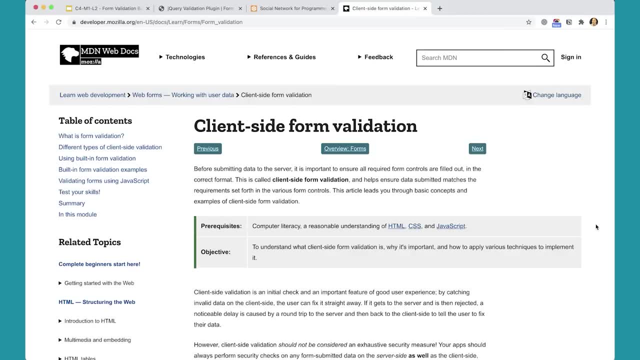 It's a great tutorial on their website And what it's using is it's taking a combination of the built in browser validation that we tried back at the beginning of this lesson, where you just put required on your input tags and do that kind of stuff. 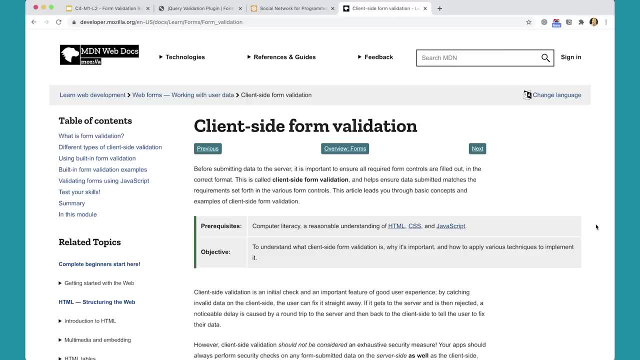 But then using jQuery to hook into the classes and the kinds of things that show up if your forms don't validate using the, using the, the built in browser validation stuff. So it uses a combination of those two things, So it's a little bit more sophisticated. 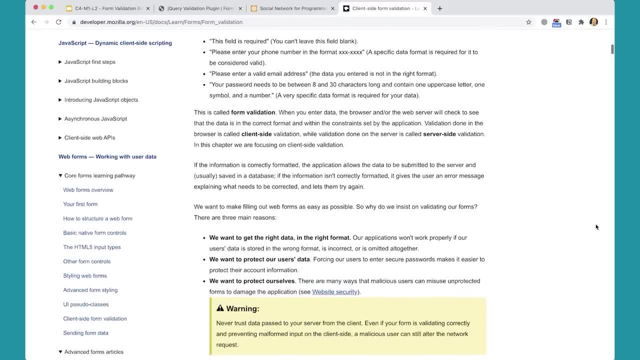 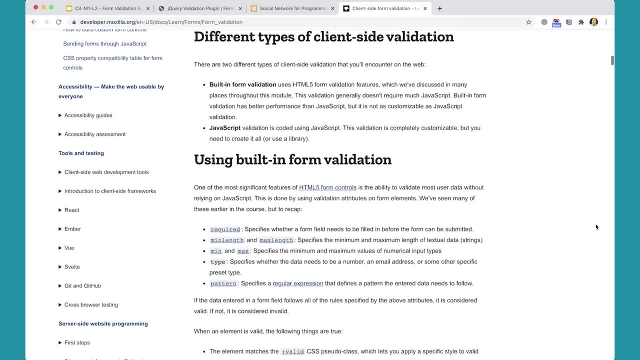 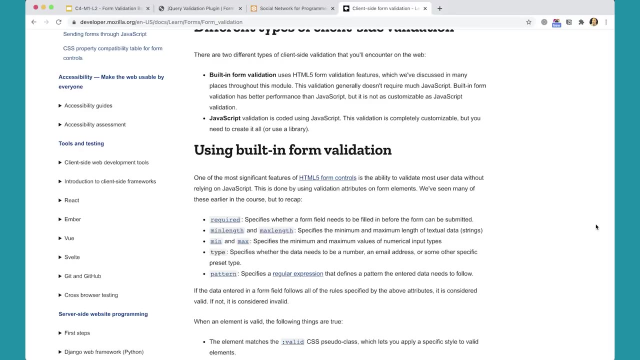 than the old school version that I showed you early on in this lesson. It's more up to date and more modern, but but it's still pretty tedious. I think ultimately you're better off using some sort of library to do form validation. But if you really want to get into 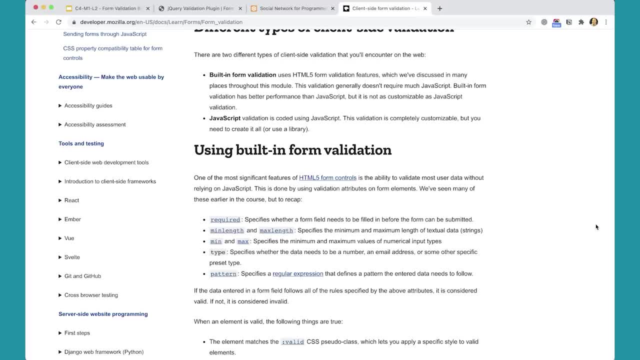 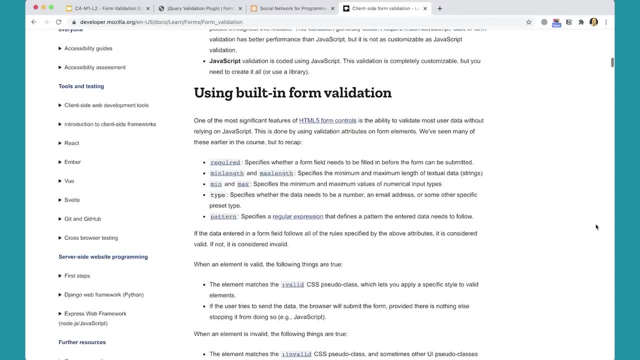 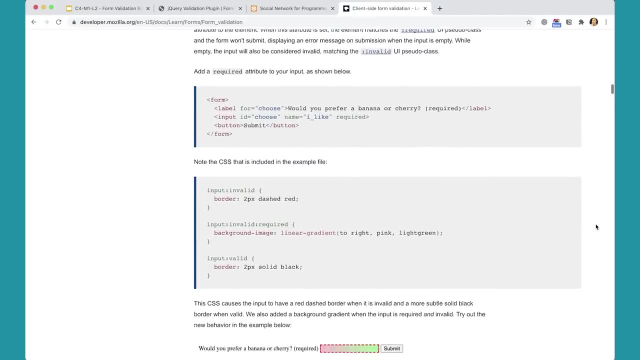 all of the power of native JavaScript and just doing it yourself, rolling yourself from scratch using native JavaScript, then this tutorial might really help you sort of look at kind of a more modern way of doing that than what I showed you. I'm going to focus on using the validate validator plug in for jQuery and show you. 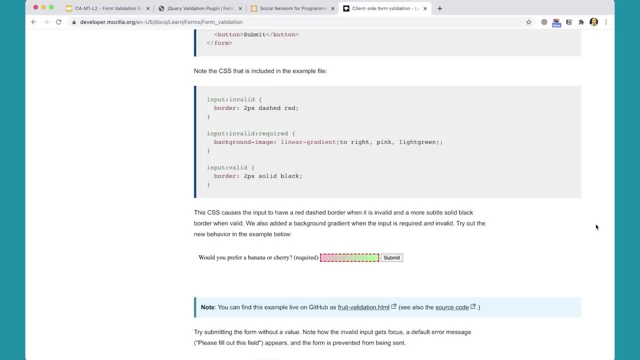 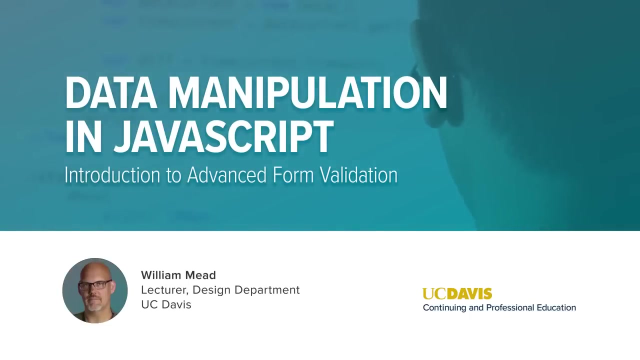 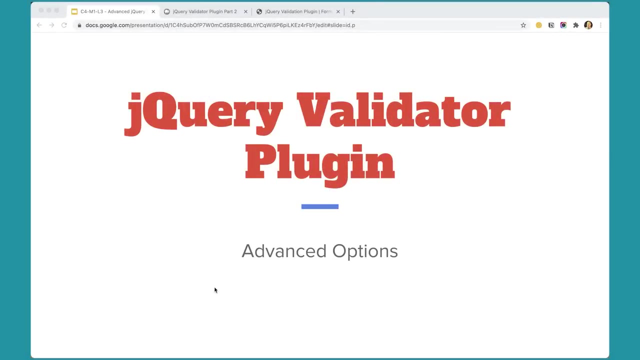 some of the more advanced features there, But there's a lot out there to explore And I strongly encourage you to go check some different things out and see which one you like to work with. The jQuery validator: plug in advanced options. In this lesson, in this exercise, we have a more. 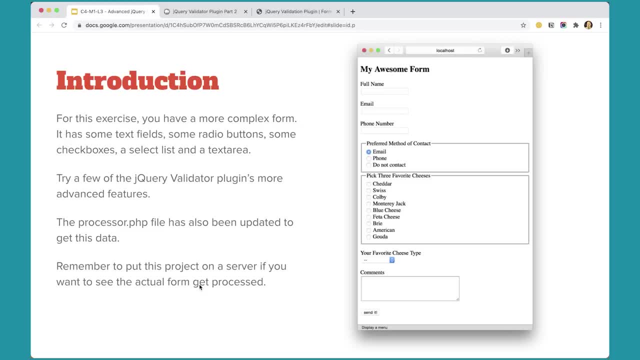 complex form, as some text fields, some radio buttons, some checkboxes, a select list in the text area, and we're going to try out a few of the jQuery validator's more advanced features, just so you can see an example of how they work, 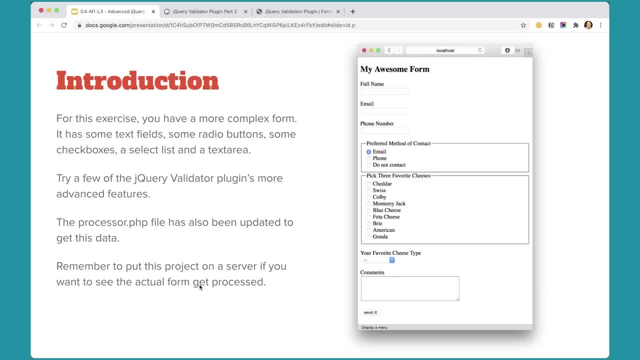 The processorphp file has also been updated to get this data. Remember that if you want to see the processor actually process the data, you have to put this file on a server or in localhost. You can run a local server by using XAMPP or XAMPP or WAMP or one of those. 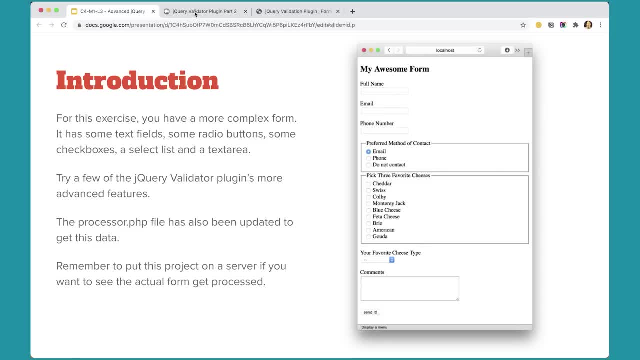 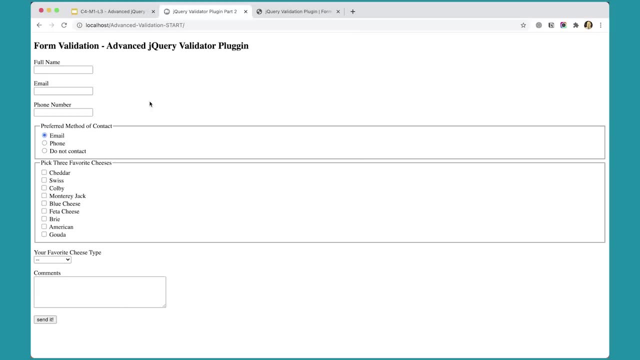 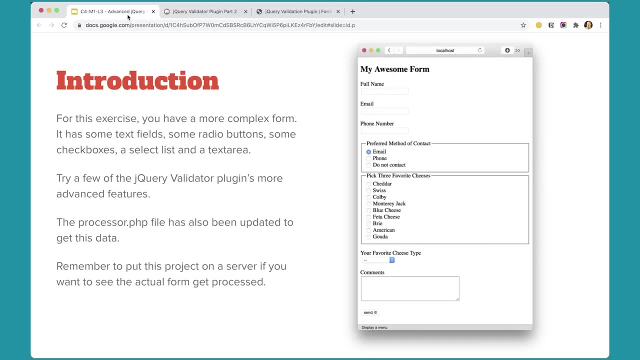 I'm actually running it through MAMP at the moment And I can come over here and you can see it says localhost here. So this is actually running through my localhost server so I can actually see the PHP get processed. But if you don't want to deal with the server side at all, that's fine. 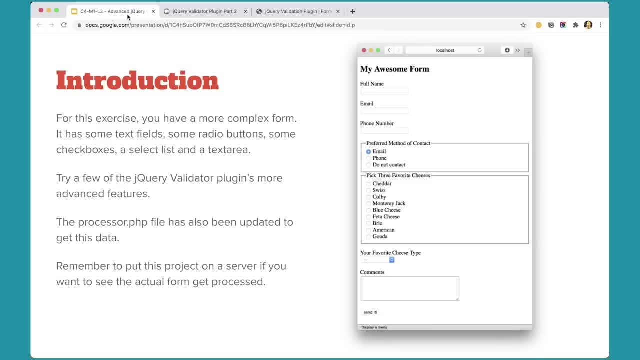 We're really going to focus on the front end and the form validation and the JavaScript involved with making that work, and the server side stuff isn't all that important to this lesson. So if you don't want to bother with it, you can skip it and just run it locally in your browser. 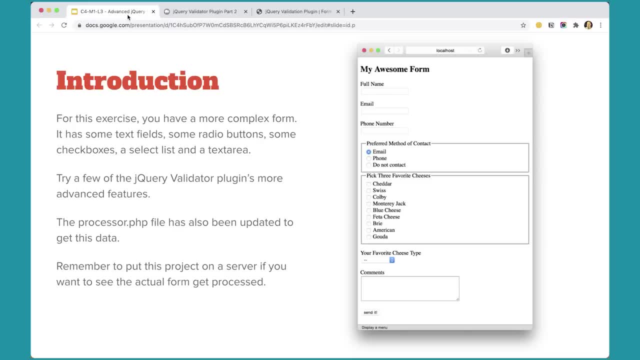 It's just when the form goes through, you'll see a bunch of PHP come through with it, which is is not really what you would get on a real server, But that's OK, All right, Great. So with that we can take a quick look at our files here. 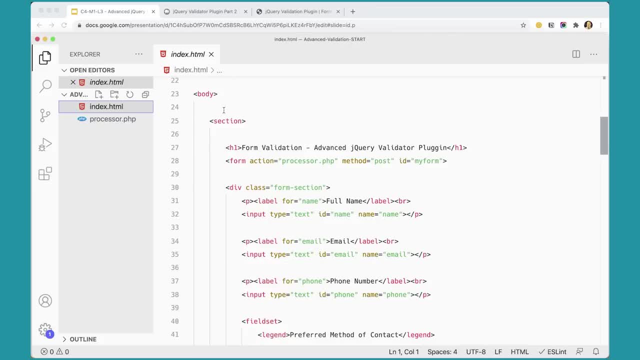 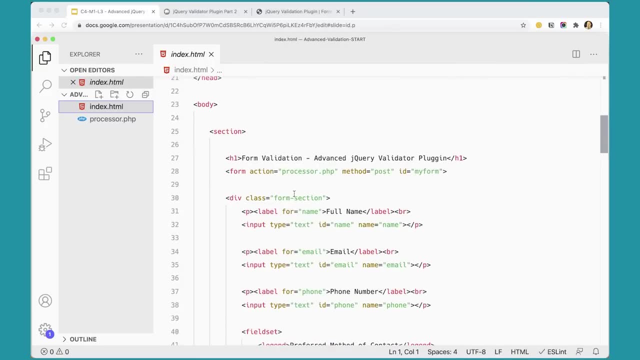 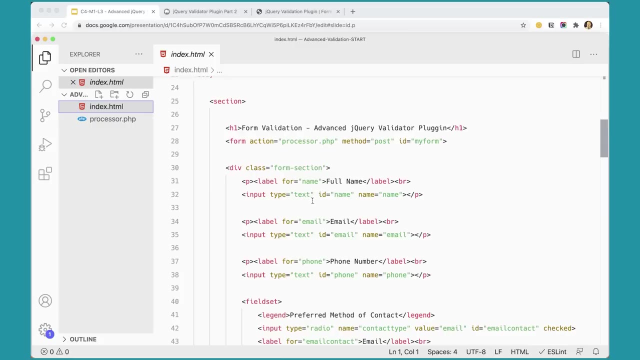 Switch over to the code editor here and here I am in Visual Studio Code and these are the files And if you look at the indexhtml file, you can see that there's already a form on the file And it's pretty straightforward. Some paragraphs with labels and input elements in here. 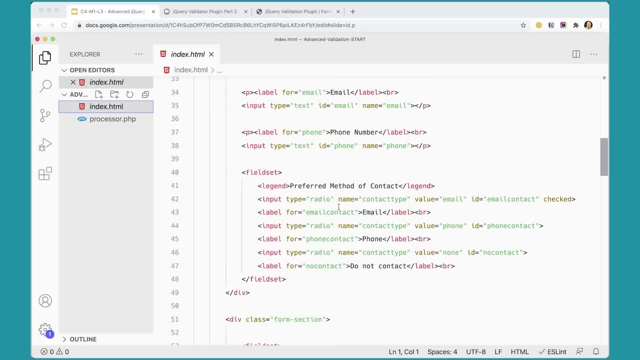 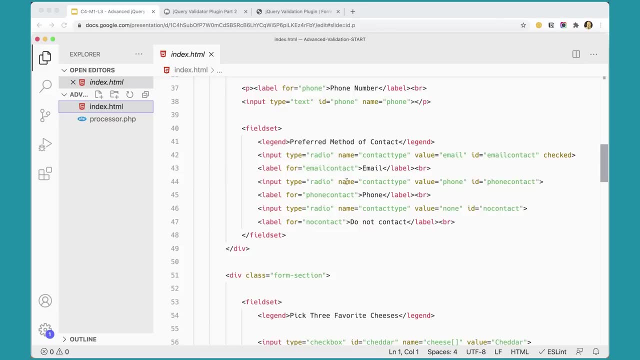 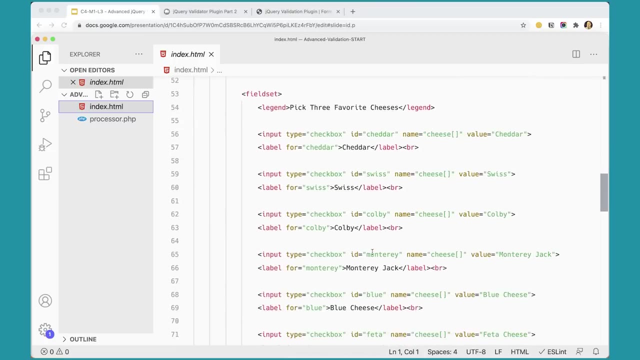 So we've got some text, one that's text, one email phone which is really just type text, And then down here we've got some radio buttons and some checkboxes. One thing you might notice that's a little bit weird about the checkbox is 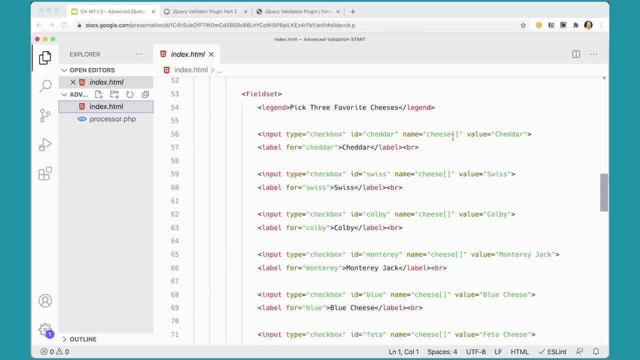 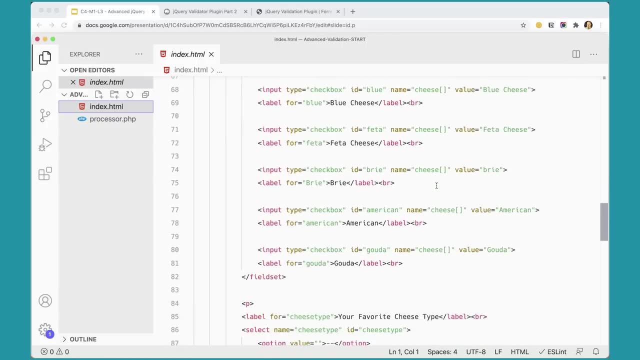 these square braces here, and this is because we're going to be sending this through to PHP as an array and then dealing with it on the, on the processor, with as an array here. So we've got a bunch of checkboxes for cheeses and then we've got a select list. 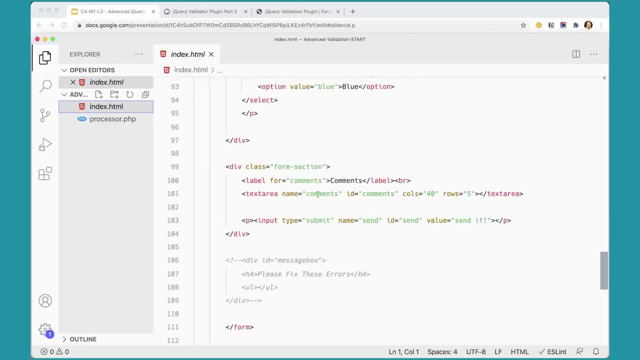 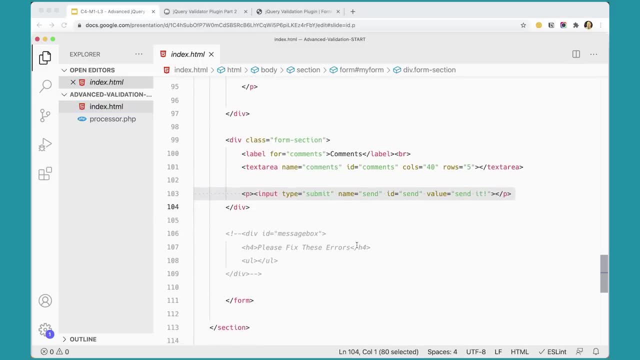 And down here we've got a text area for comments and then finally, our submit button that we need to submit the form, And that's the basics of what we have for the HTML for the form, And there isn't, doesn't look particularly good. 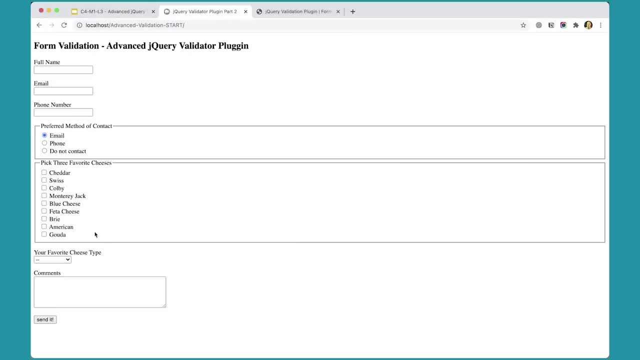 There isn't any styling at the moment, So it all just kind of looks like this. but that's OK, OK, great, So we've got that in place. The next thing we need to look at really quickly is just the processor, PHP file. 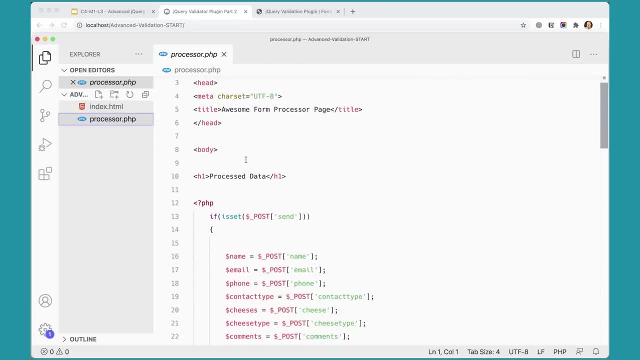 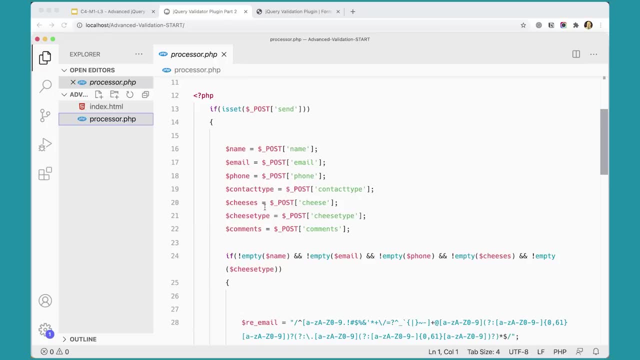 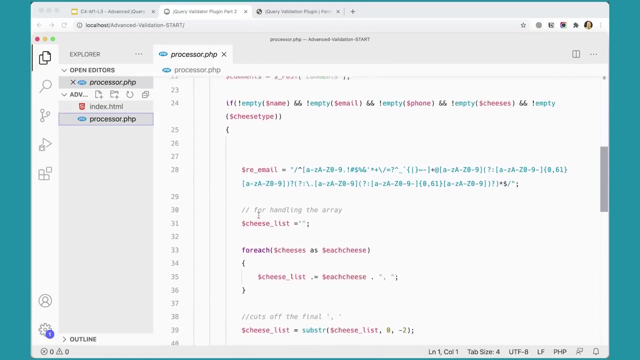 So you can see over here really quickly. We're just going to get these pieces of data from the form. You'll notice that when this one comes in, this comes in as an array. So I have to- first I'm going to check to make sure they're not empty and all that kind of stuff. 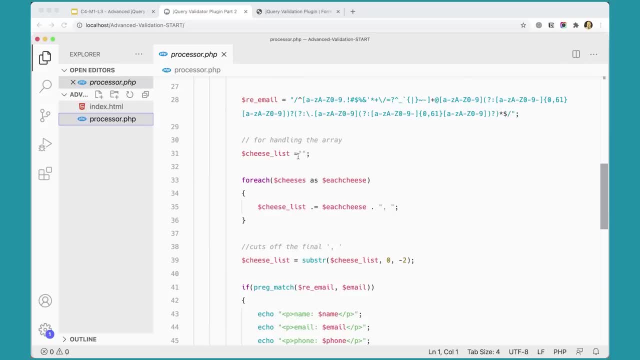 But for the array of of cheese list, I'm going to set an empty string here and then just loop through each of those elements in that array and put them into this list, followed by a comma and space, and then I just remove the last comma and space. 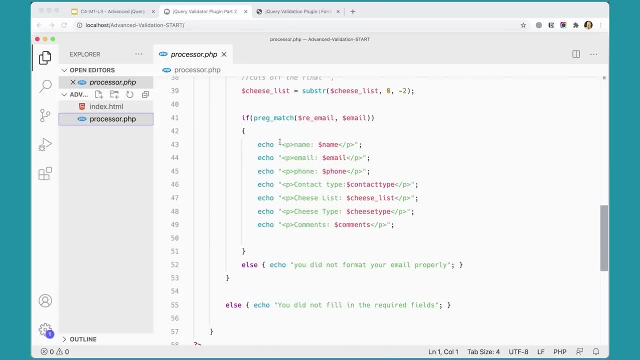 at the end and do that kind of stuff, And then I'm just basically assuming everything matches and everything's good. I'm just printing this stuff out to the screen, But if something goes wrong, then one of these other else statements will run. 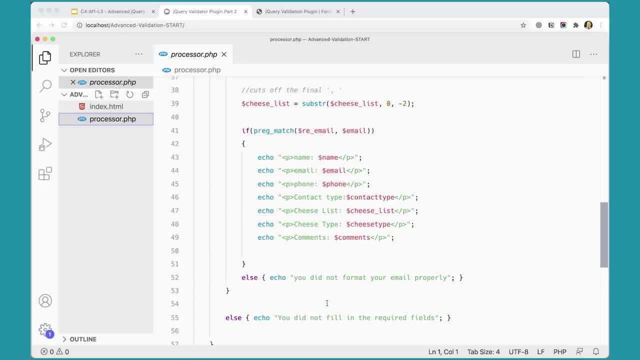 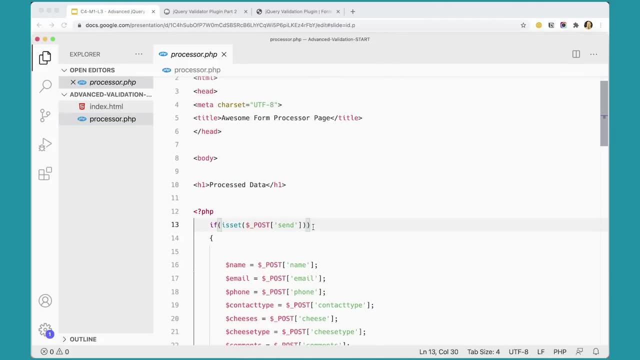 But we're going to catch all of those. None of these should run because we're going to catch all the all of that in the JavaScript on the front end. In the next video we'll look at getting our script started and getting everything going on. 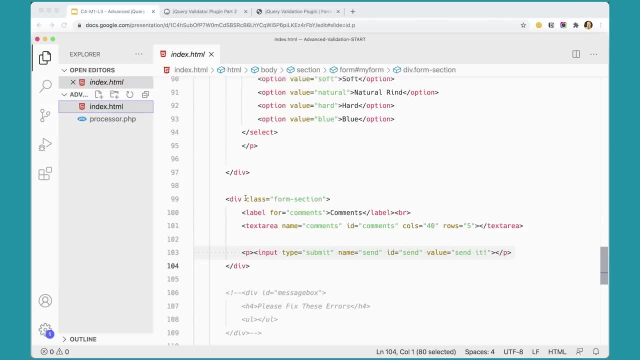 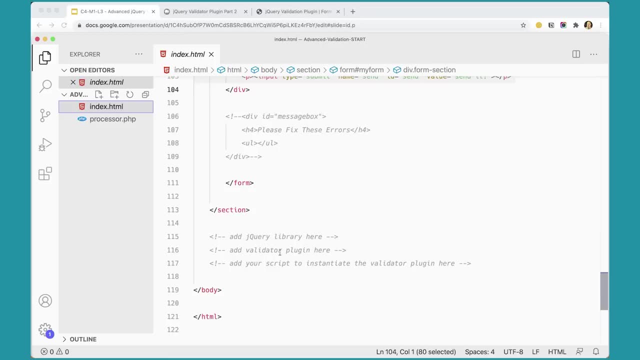 We're going to have to get our index HTML files that we're ready to capture to our validation and capture the stuff, And to do this we're going to have to hook up the jQuery library, the validator plugin, and then add our script for initiating the validator here. 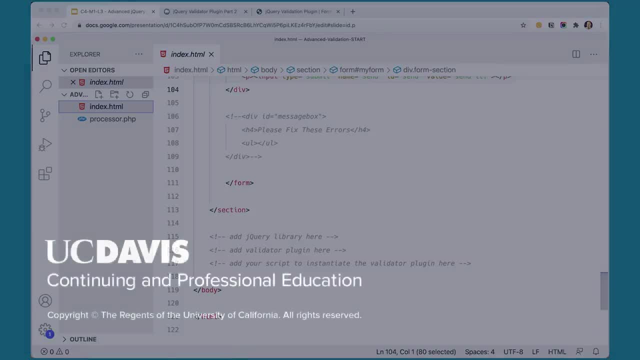 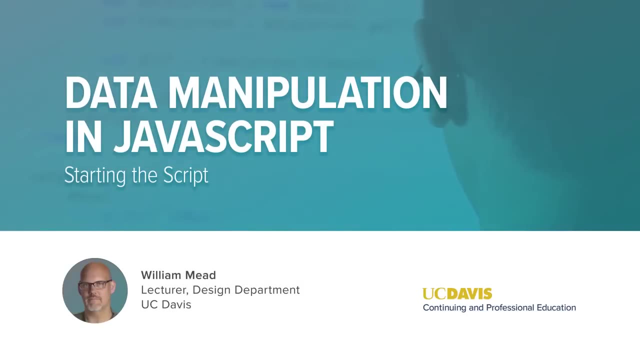 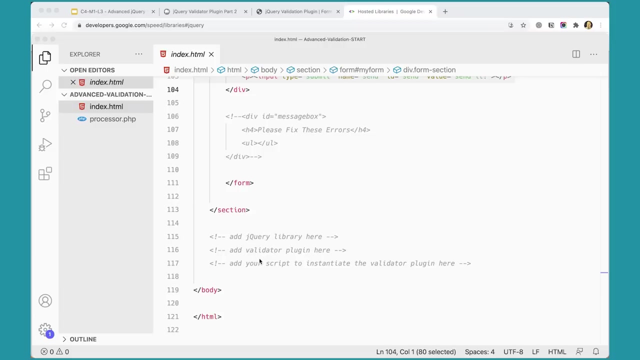 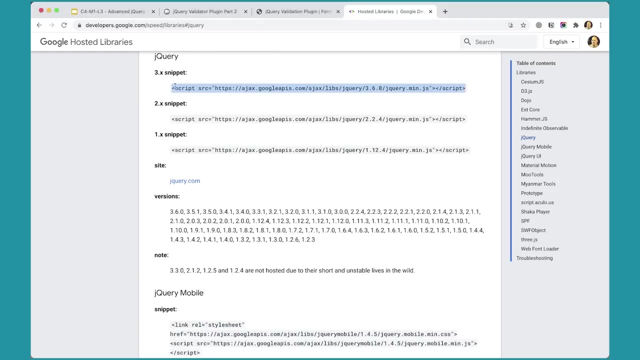 Or you could put it in an external file if you wanted to. Now that we've introduced the project, we can get our script going and start initializing everything and just start with. I need to add jQuery here, And so I went over to the hosted libraries on Google and I. 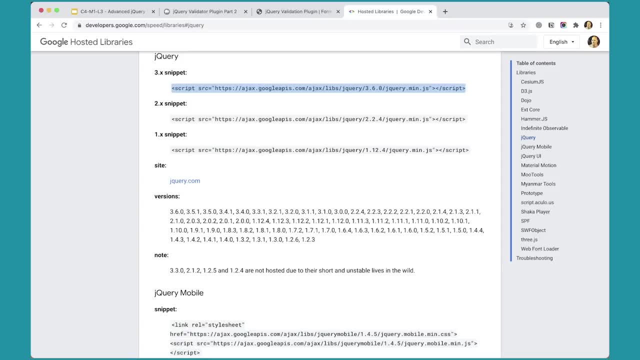 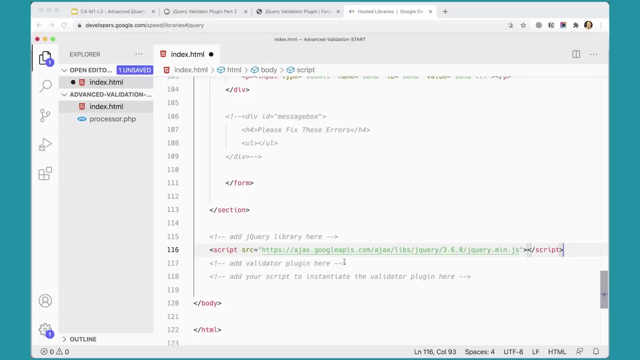 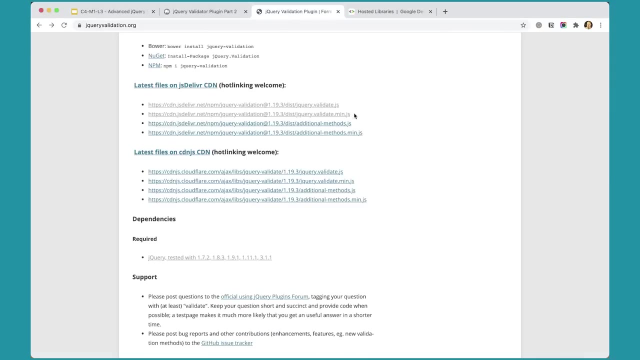 copied this snippet for the latest version of the jQuery library And I'm just going to paste that link right in here, Like that. And then we need the jQuery validator plugin. So I'm going to go over to the validator plugin website, and this is actually the one that I want here. 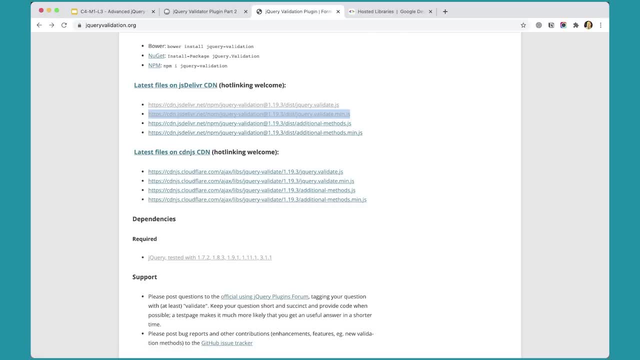 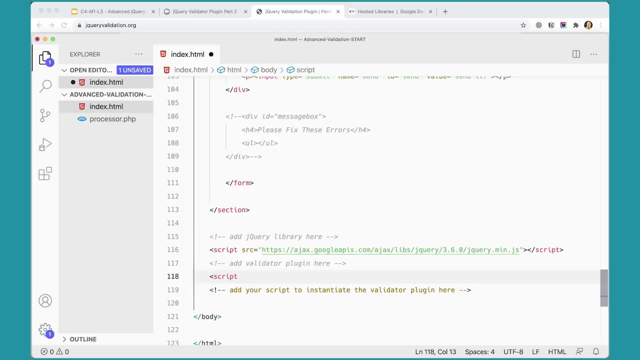 Of course it's just giving me the URL, so I have to type the script tags. So in here I'm just going to type script and SRC equals, quote, quote and paste that in and then close. the script tag Looks a little funny because I'm going to close my Explorer here. 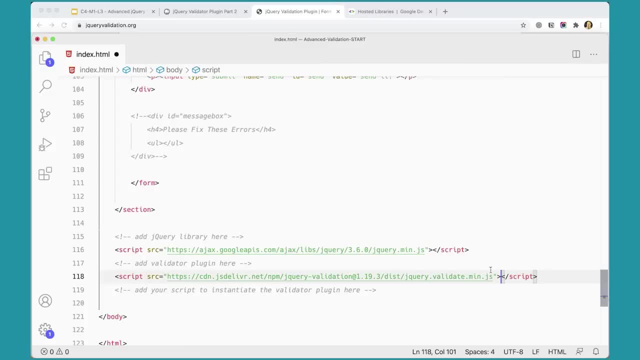 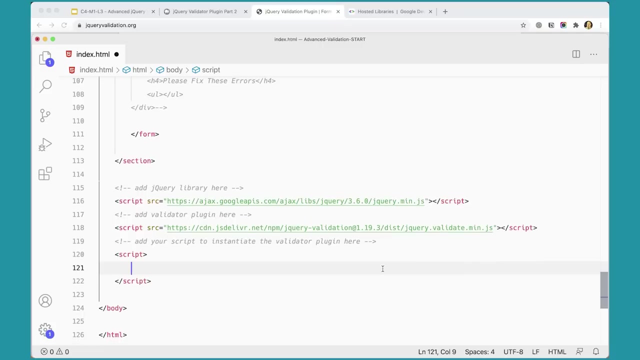 There we go, So we can see it a little bit better. So we've got the validator plugin. plug it in, so that should all work really nicely, And then we can add our script tag here And we can start working on our validator right here. 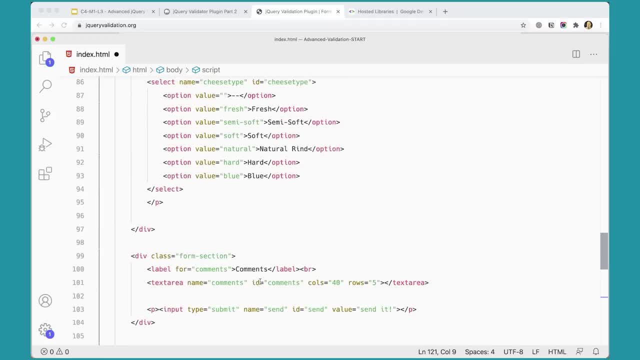 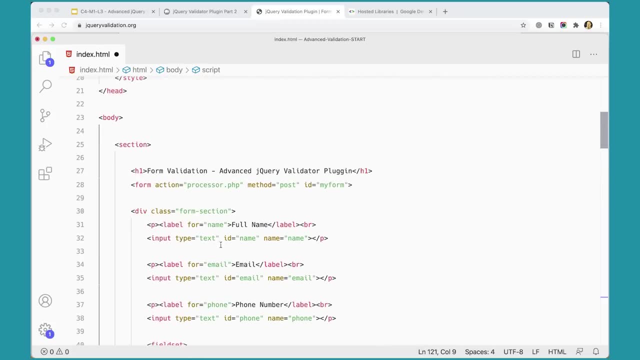 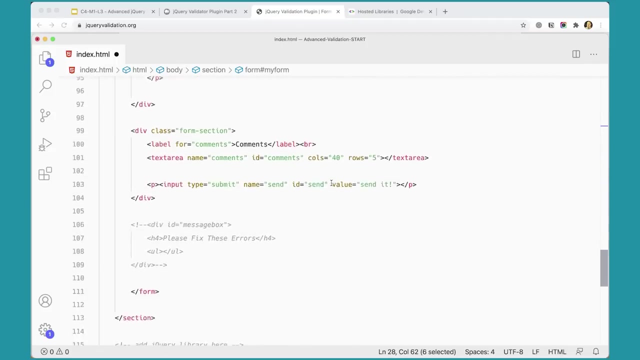 And what do we want to do? first, We want to tell our form- This form here, Where is it? Form my form, this one right here. copy that ID, Because down here we just want to say: use our jQuery object. 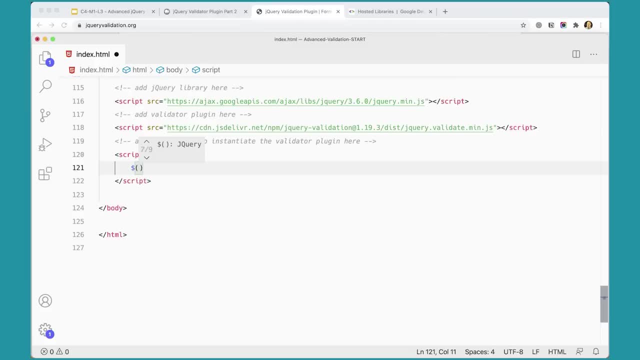 in here to get pound my form. Don't forget the hash there. Dot validate Great. So that's the basic validator. That's what we did in the previous lesson. Now, to make use of the more advanced features, we're going to pass in an object here. 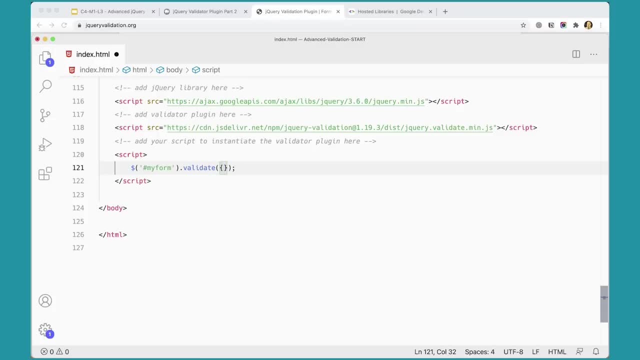 You've already learned a little bit about objects in the previous lesson. Plus, we saw the same behavior in a previous lesson when we did the flex slider plugin, so it's kind of nice that these plugins follow this familiar convention of when you want to make use of additional features. 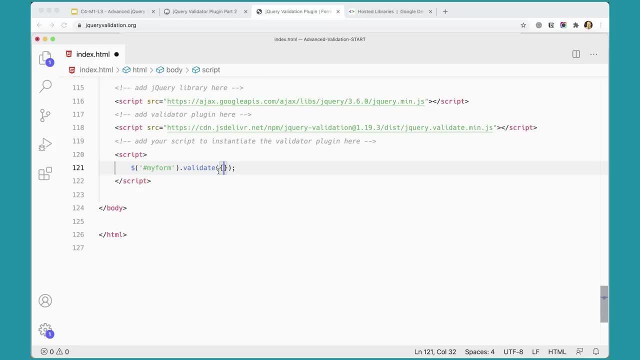 you can pass in an object and those features and settings can get set within the object. So I'm going to move that, I'm going to move this down to make some room in here, And then in here we're going to add some rules that we're going to follow for our validation. 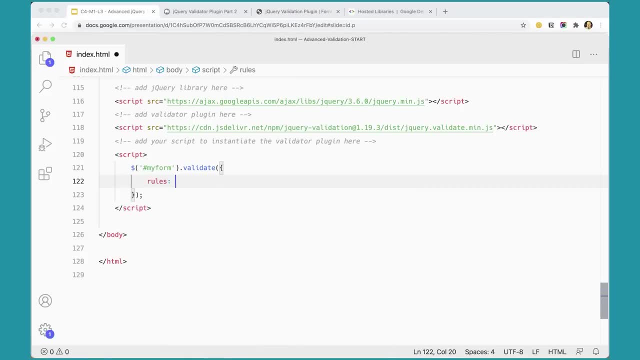 So we'll add rules like this And you'll notice that the first element in this object here is going to hold another object. So we're putting an object inside of an object. So this rules is our first element and it's and its value is going to be an object. 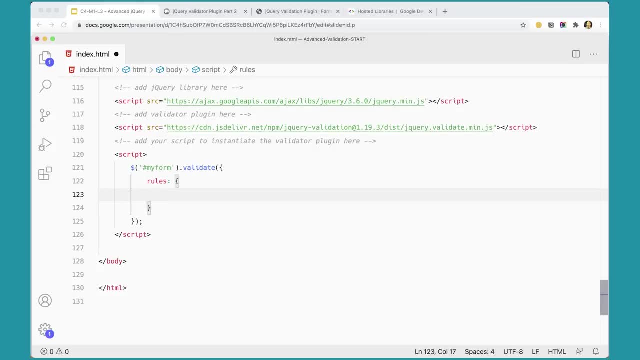 And so what am I going to put in here? I'm going to put a sub element or an element inside this element that says name. I'm going to set it to required, Like that. There we go, we're on our way. so we don't put a semicolon there, we put a comma. 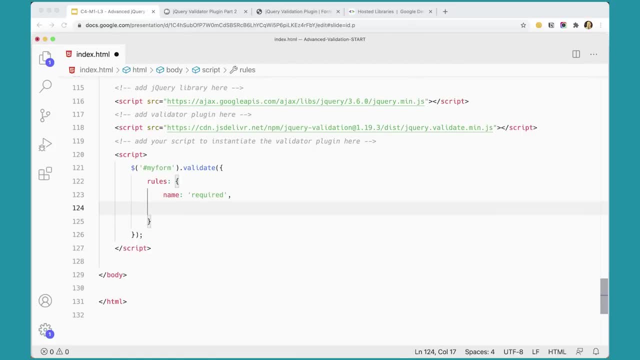 There we go. And then the next one we're going to say for email. And email needs two things: It needs to check to make sure that it is required and it needs to check to make sure that it's a valid email address. So this is going to hold another object. 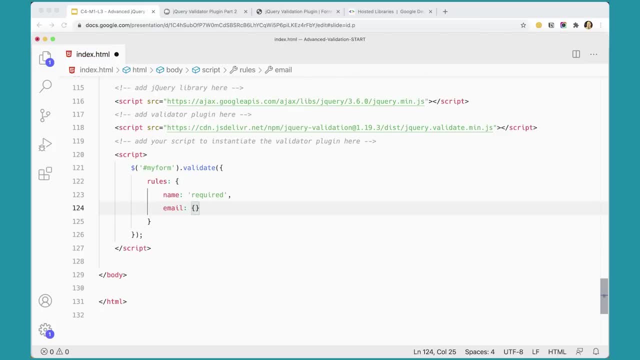 So we're putting an object inside of an object inside of an object, And I'm just going to put it all on one line here And it's going to say: required True Comma Email, True Like that. You might wonder why this required is not in quotes, but that one is. 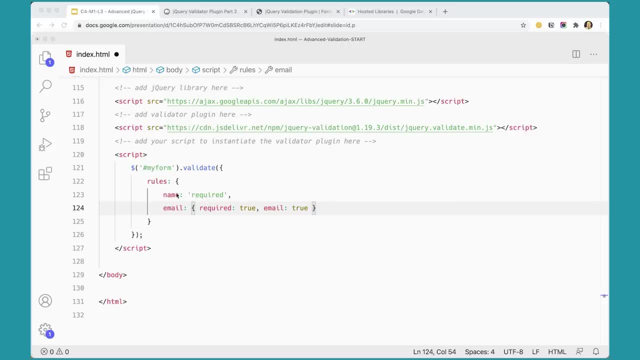 This required is a is a value that goes with this property. This required is a property and the value is true. True doesn't go in quotes because JavaScript knows what true means. This is also a property, so it doesn't go in quotes. 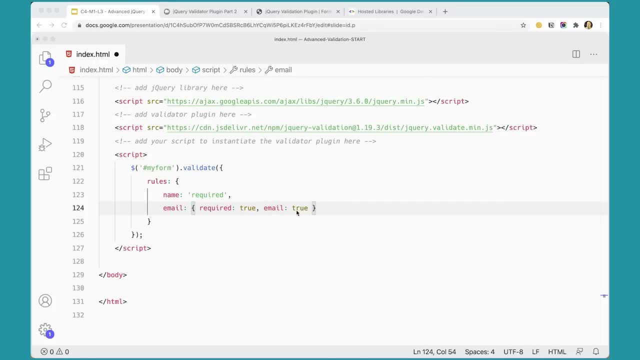 But this is a value, So it is. And because it's true, and JavaScript knows what that is, it doesn't go inside quotes, All right, So we've got that, And then the next thing we need to do is put a comma and go on to: 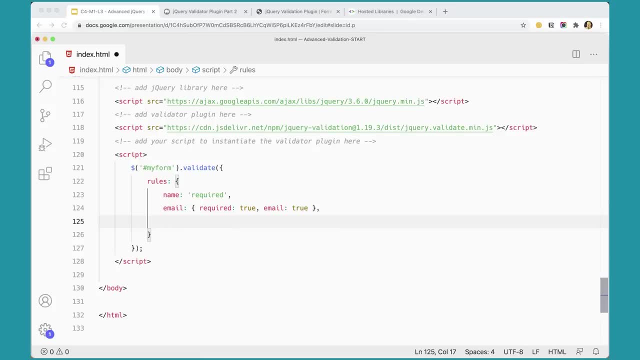 Validate the cheese array. So to validate the cheese array. Now, this one's a little bit different, because, because cheeses, it would look like this: cheeses, cheese, cheeses, I think, square brackets Like that. Actually it's just cheese, not cheese, it's cheese. 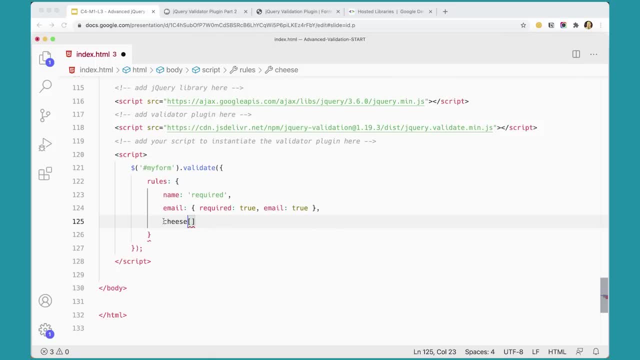 It would look like this, but because of the square brackets that's going to cause problems. So we actually have to put This particular property in quotes. So it's going to go like that, and then we'll have the semicolon, And here we're going to again put in an array. 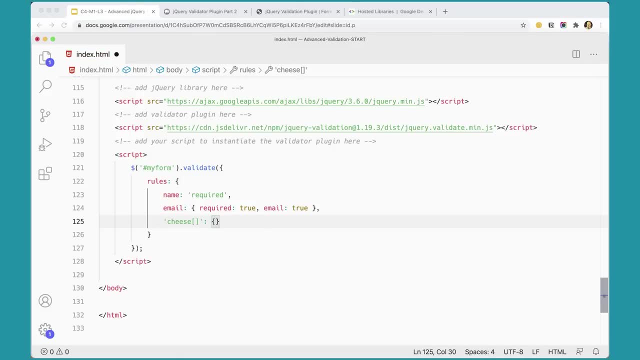 I mean not an array, an object. And this object is going to have a few different things. First we're going to say that it's required, Required, true. Then we can actually say that we want a minimum and a maximum. 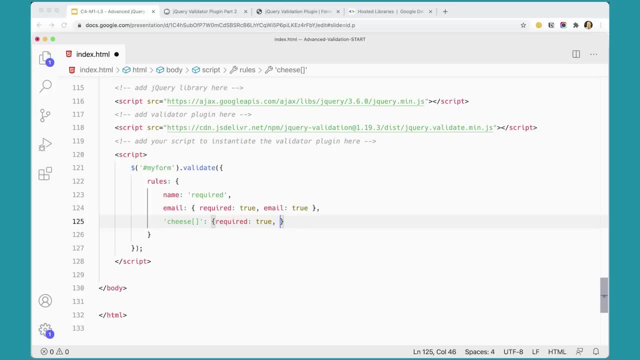 Number of checkboxes. So if I want exactly three, I can set the minimum to three and the maximum to three, And then I'll get exactly three options. We do that by setting min length. Make sure you spell length right. I always spell that one wrong. 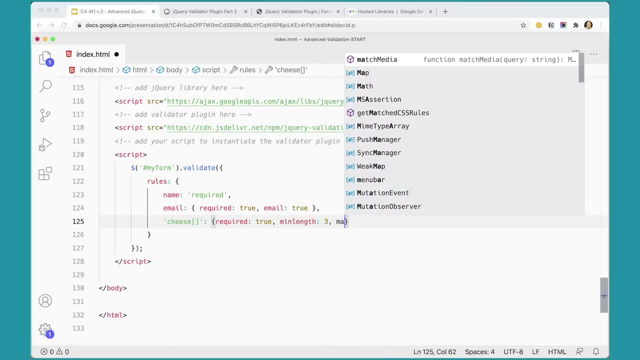 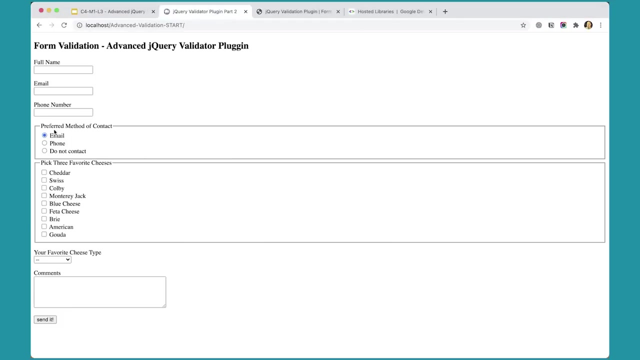 Min length three And max length Three. And again, JavaScript knows these are numbers, so it knows what to do with those. And now we've got our, our rule for what we're expecting over here on our: In your pick three favorite cheeses. so you have to pick exactly three. 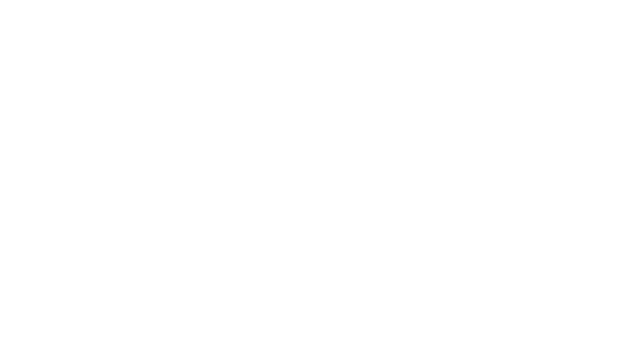 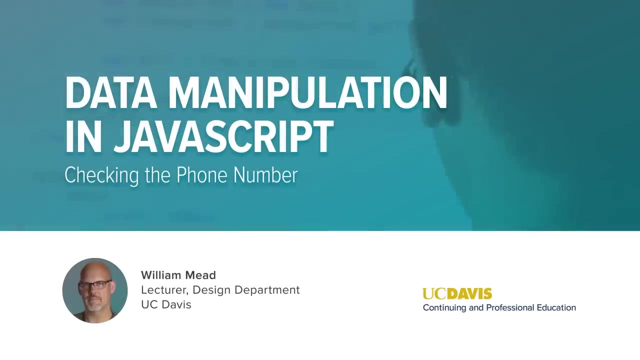 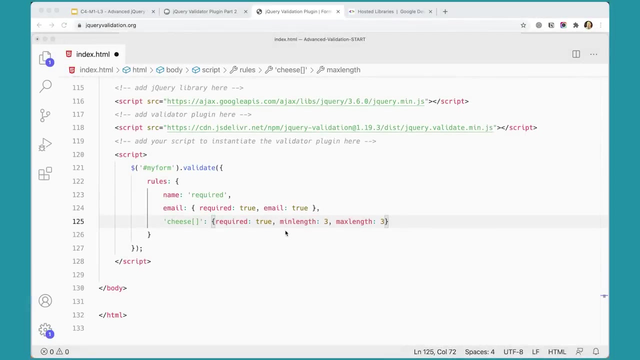 So that will work for that now And that's what we want Now. In the previous video, we got our script started, We hooked up our jQuery and our jQuery plugin and we started writing our script here And next. the next thing we need to do is we need to. 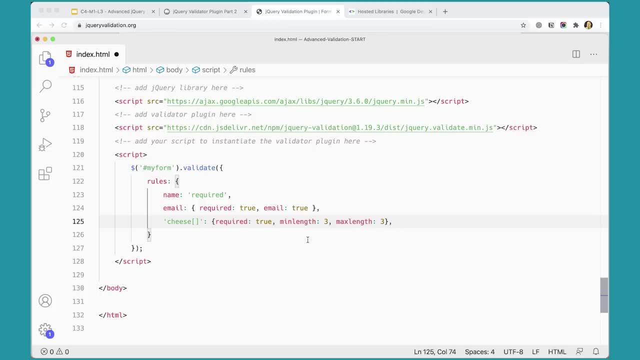 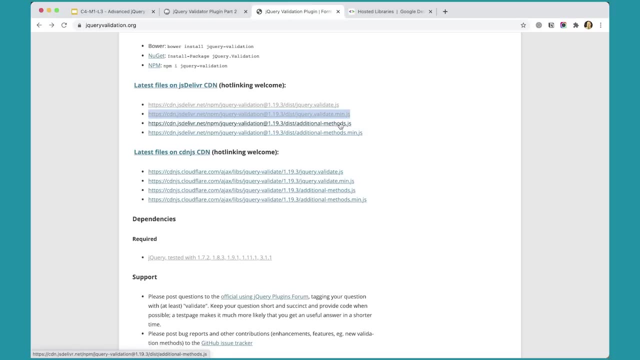 and what type of phone number you want to validate. Now, if you go to the jQuery validator website, there's this additional methods plugin that you could add And this additional methods- one of the things that it includes in there, I believe, is a method for checking US phone. 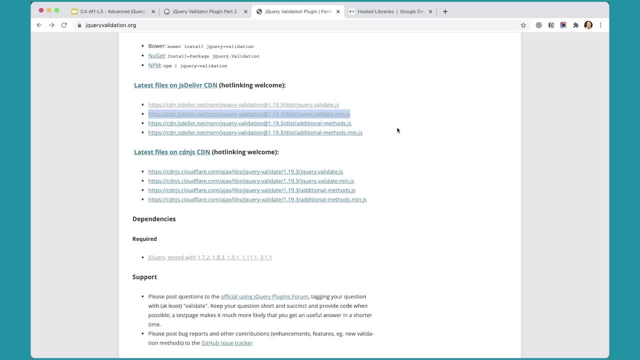 numbers, But also one of the things that's really neat about the jQuery validator plugin is you can add your own regular expressions for it to check against as well. So I have a regular expression that I use for checking US phone numbers And you could find one for checking. 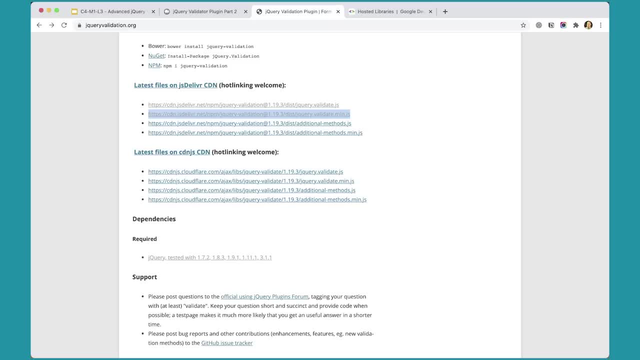 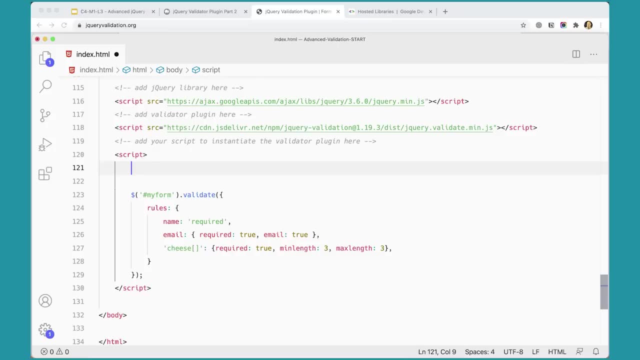 phone numbers in a different country if you wanted to. But I'm just going to paste it in here And I'll provide this for you so that you have access to this one. And I'm just going to paste it here Because this is not something you want to type. 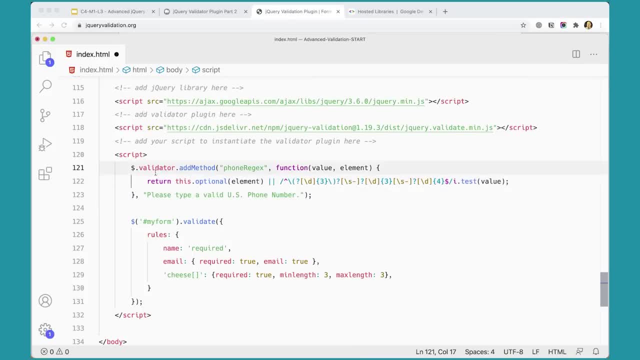 But you can see, here I'm saying validator, add a method, And I'm calling it phone reg X, And then I'm passing in a function with a value element And it returns this optional element, which is a regular expression, And it has a message: please type a valid US phone number. So you 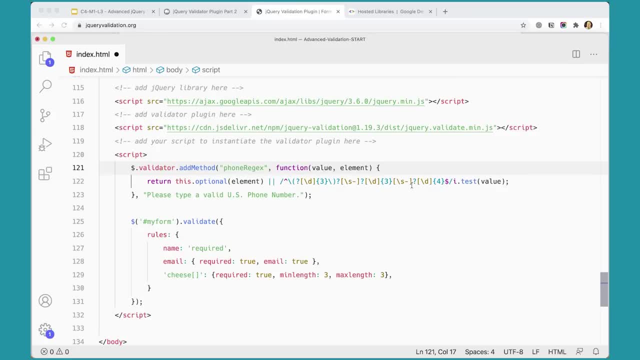 could change this regular expression to something else. You would change this part of the expression here from here over to here. You would change that to something else if you wanted to check a phone number in a different country, And then you could also change the message down here. 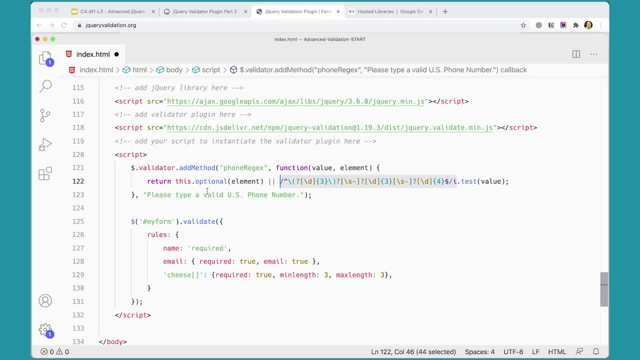 But it's pretty neat that we can add in additional regular expressions to check things in our validator plugin this way. I think that's a really neat feature of this particular validator. So now that I have that here, I can come down here and add phone. 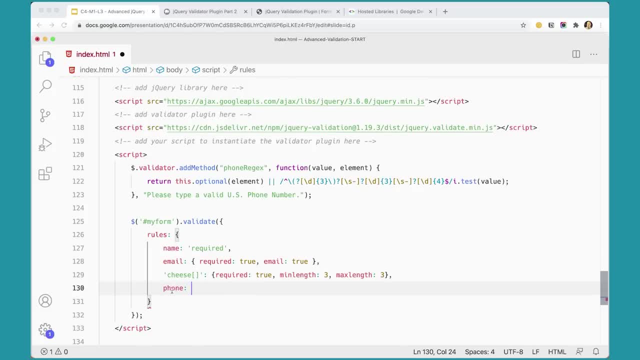 As a property and the value is going to be another object. Required: true, true comma. phone reg x. this label here is matching this phone reg x up here and let's set that to true as well. great, we've got that in place. the last field that we're going to require: 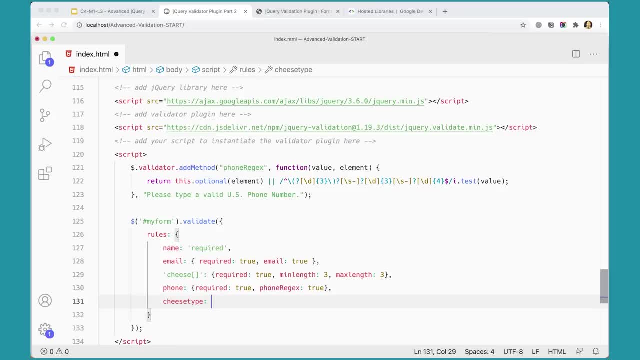 is the cheese type field and we're just going to set it to required like that. no comment at the end of this one. because this is the last one and really, what is this field if we come over here? it's this field here, and because it's a select list. 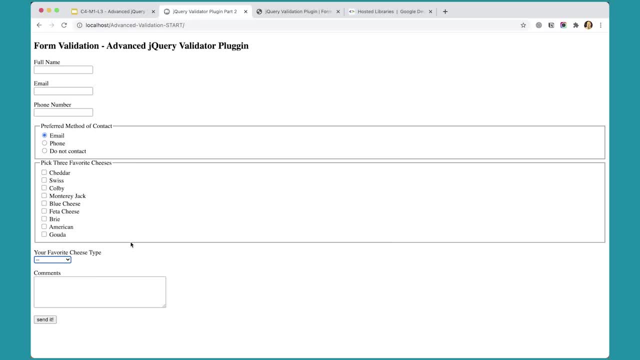 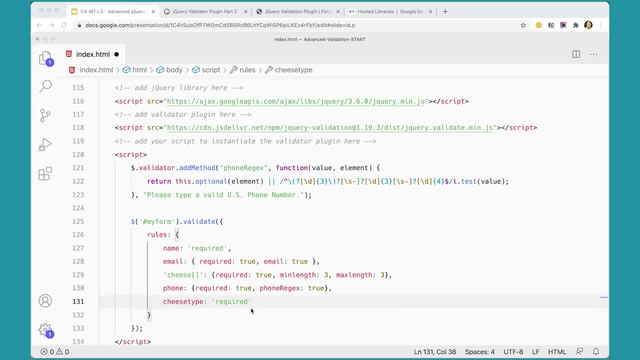 you can only pick one from the list, so we're just going to require it and that's fine. now, if I've done everything right- which is a big if always, we should be able to save this file here and then come over and actually test it. if I refresh my page here, 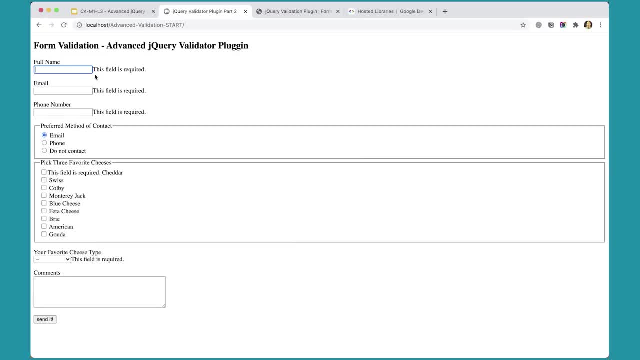 and it should. it should kind of work. we're just getting generic messages here, but it is actually working. you know, it says this field is required, you know. so it is putting these in here, but it's it's not. it's not doing anything great with it yet. 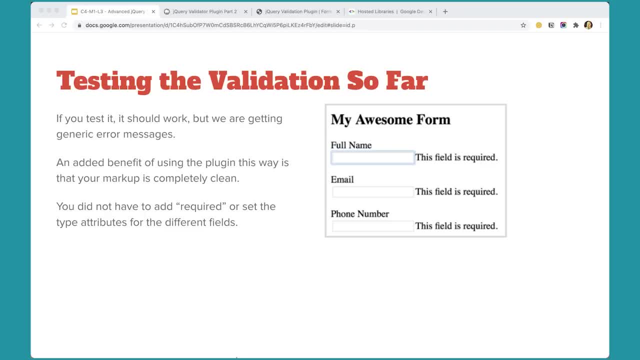 so we need to do a little bit more to clean this up. one of the really nice things about this plugin is that you'll notice that our our markup is very clean. we haven't had to add the required attribute. we haven't had to add anything extra to our html markup. 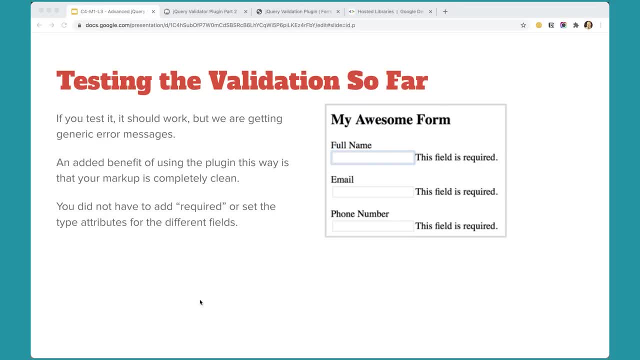 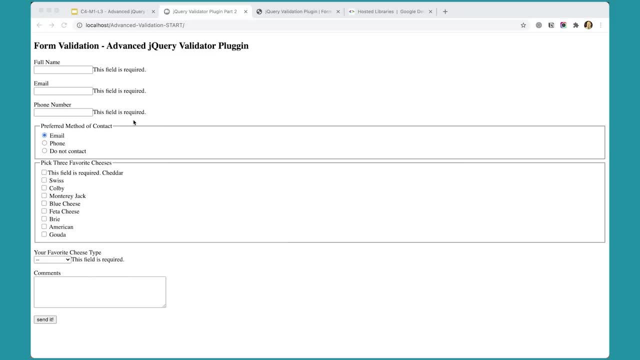 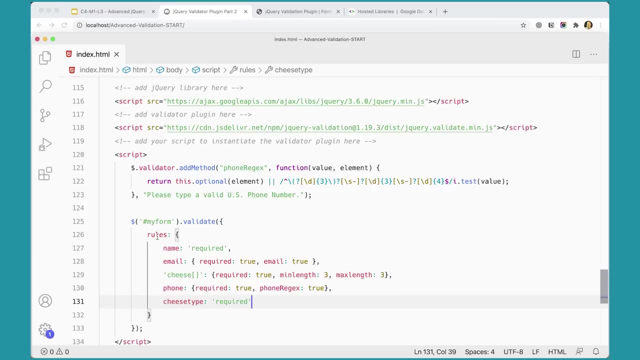 everything is being taken care of in the javascript, and that's really pretty nice to improve the messages that we have here. we'll just go back to our code editor here and after our rules property, inside the main property for our validate plugin here we're going to add a comma. 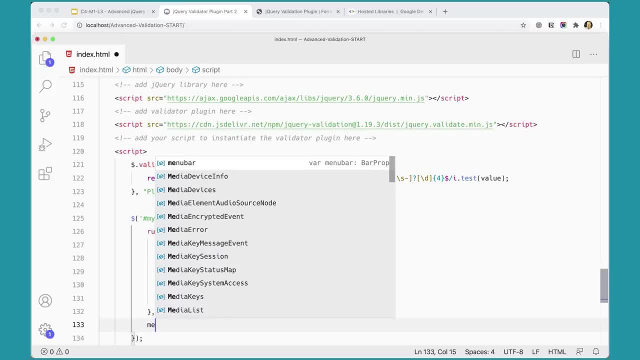 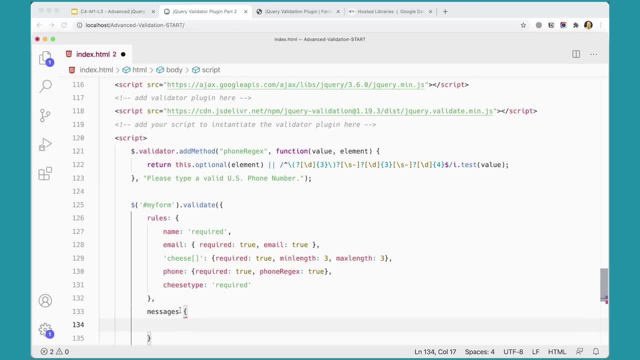 and then we're going to add messages, and messages is going to be another, is going to have another object in it, just like rules. so this is the second property that's at the root level of our, of our thing here and then of our validate function here. 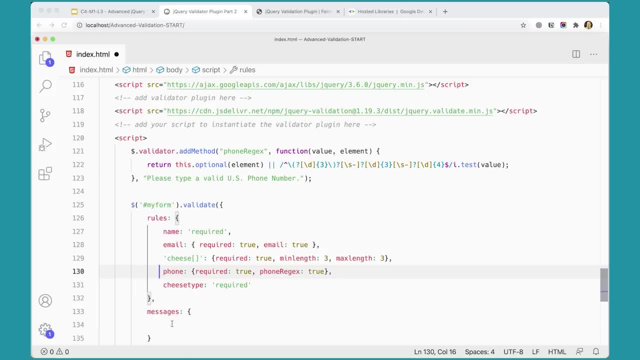 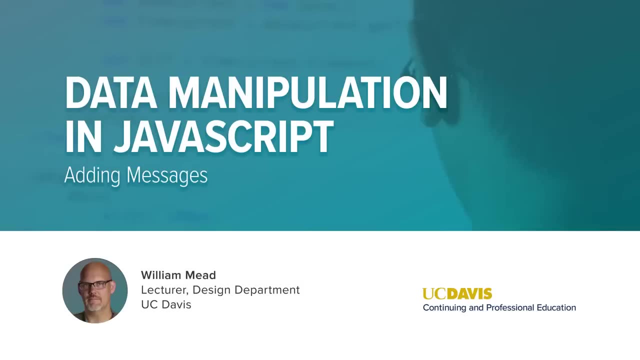 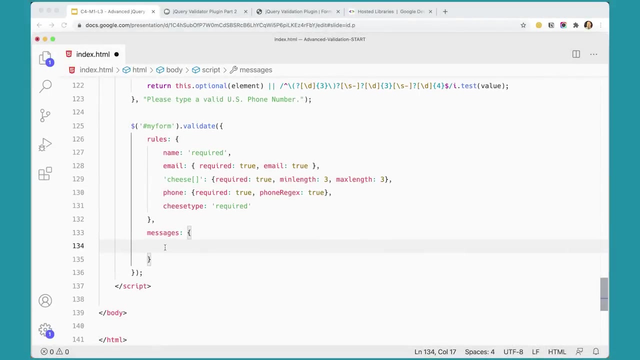 and then we'll add some messages in here in our next video. if i remember correctly, just as I said, just like after not landing in this page, we were even now. so we're gonna be adding in some filters and we're gonna adjust asius. so now we're ready to add some messages in that will be custom for our design here for our page. 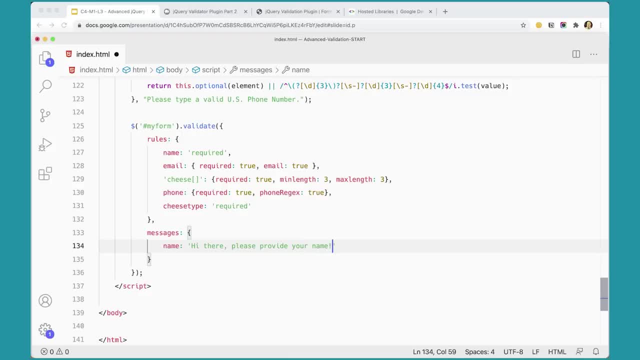 and so the first one is going to be for the name field, and i'm just going to put in something like: And you can set these messages to be whatever you want them to be. And that's one of the really nice things about this plugin is that you have full control. 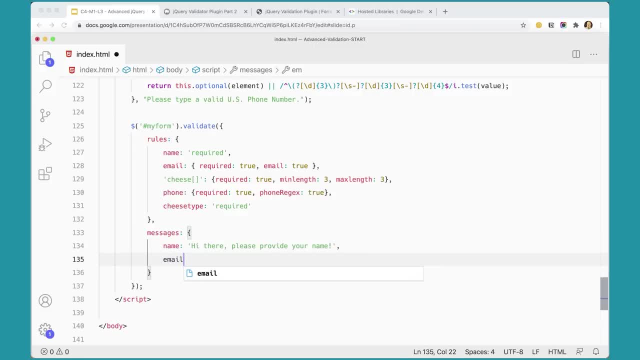 over all of the features. The next one will be email, the email property, And again, because we're doing two things here, we need two messages for the email. So that's going to hold an object And the first message is going to be for the required property. 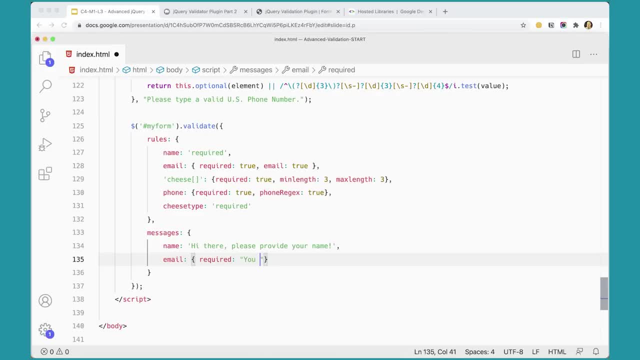 And we'll say it. you know. say something like: you must provide an email, And then the next one is going to be for the email property. Okay, A valid email address, please, Something like that. And then we've got a comma. 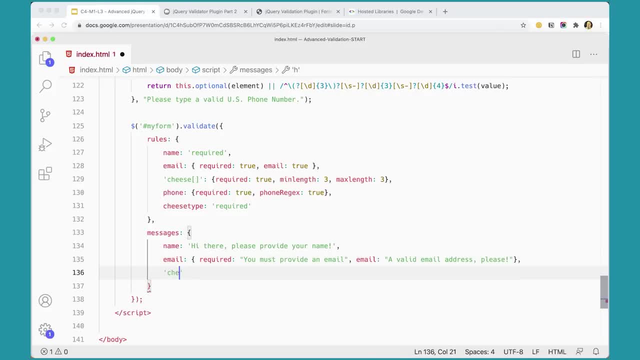 And then next we've got our cheese with this. This one goes in quotes because of the square brackets, because it's an array, And this one is simply going to have a message that says, Okay, Please select three cheeses, something like that. 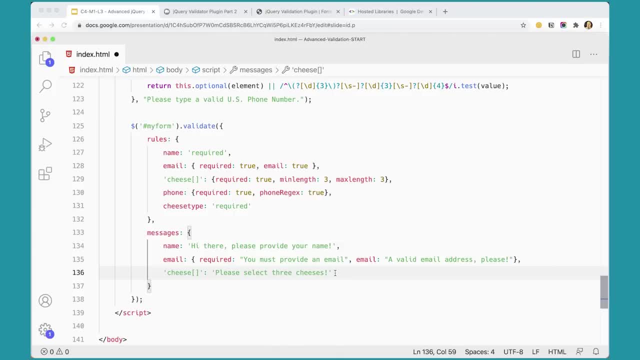 For phone. we're going to have an object- again whoops object like that- And we're going to have the first property in this object is going to be required And it's going to say something like this. And it's going to say something like: please provide a phone number. 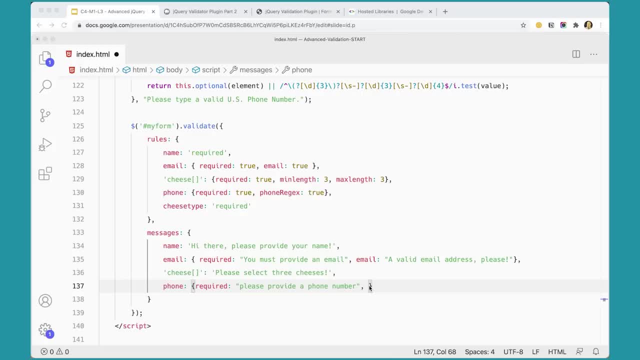 And then the second property is just going to be phone And we're just going to pass it an empty set of quotes, because really, what's going to go here is this: Okay, Okay. So the first part is this one up here. 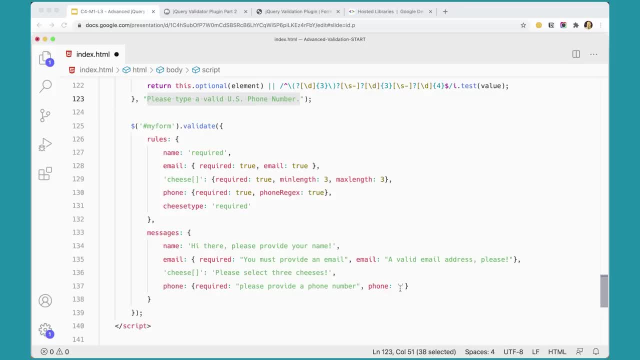 So that's going to be the message that gets passed in here. So we're just putting in an empty set of quotes there. Now, if you're wondering how I know all of this and how I kind of figured all of this out, it's really not too difficult. 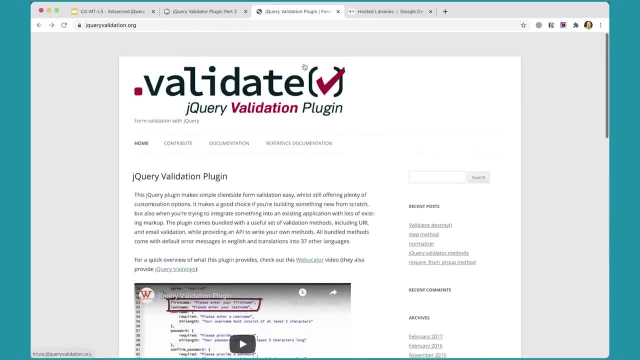 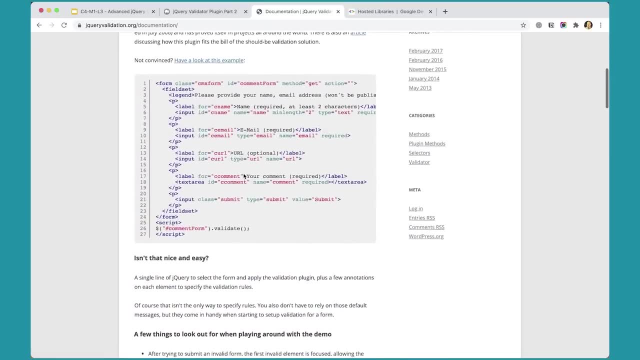 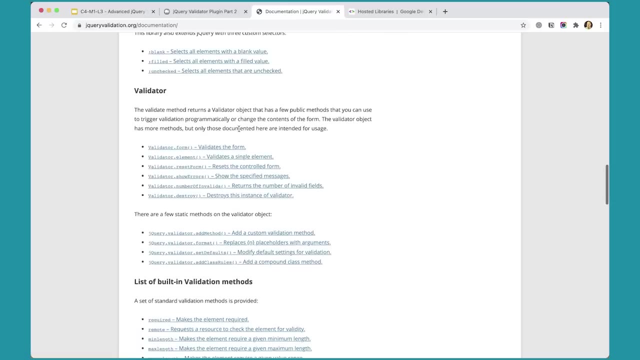 Over on the jQuery validator plugin website. if you go to documentation. I did all of this in just an evening of looking through the documentation on this website. they provide examples, Okay sorts of really great information about how it works, and you just have to poke. 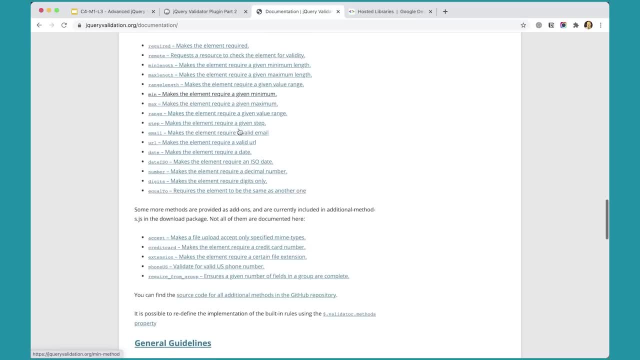 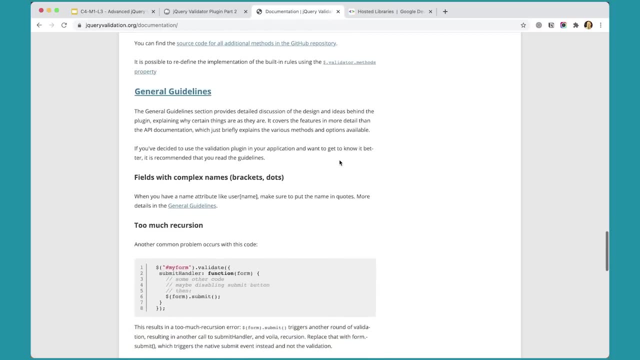 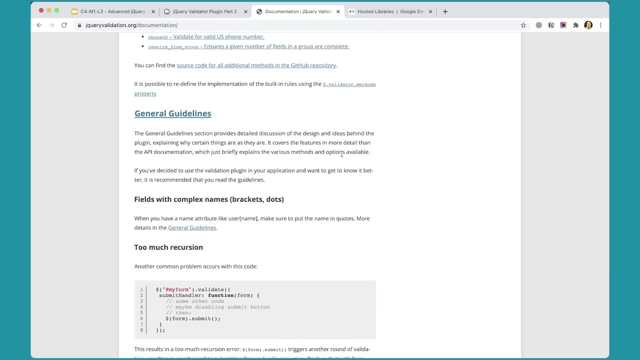 through and look at some of the different methods and things that you can do, things you can check and all of this different kind of stuff. it's all in here and you can find lots of things that that I haven't done in this example and you can play around with them and do some fun, interesting things here. let's 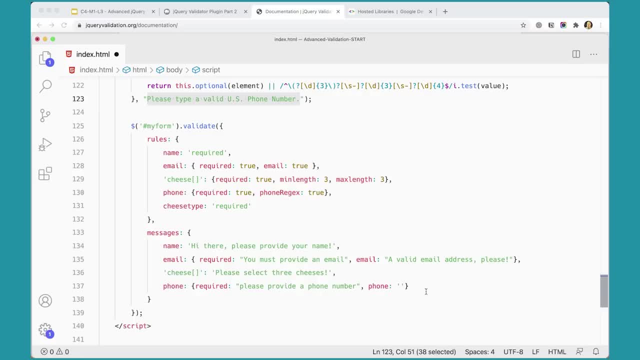 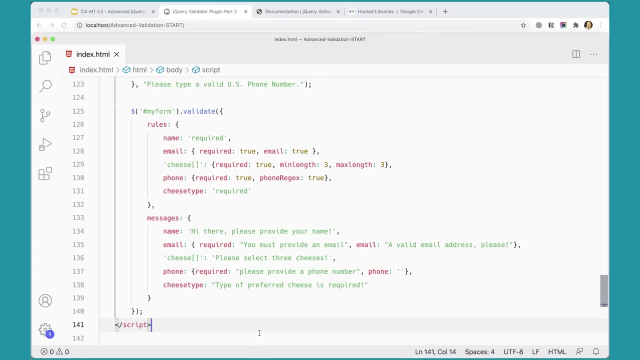 go back to our code editor and add one more. for cheese type, type of preferred cheese is required exclamation point. and there we go. now we have our messages. at this point our validator should be working and we should have some messages going and it should all be good. let's give it a try. assuming that I typed all. 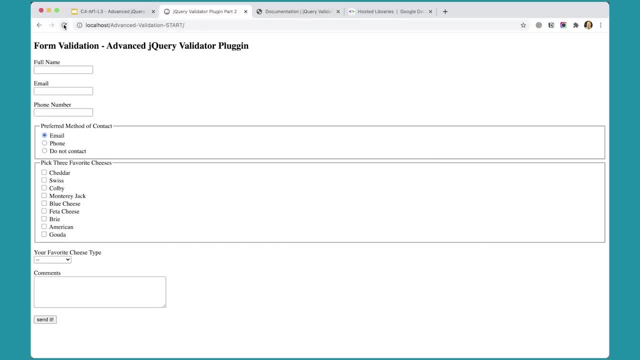 of this right, and maybe I did. sometimes I make mistakes, we all do so. if you make a mistake, go back and check everything. but I'm going to just refresh this and then click send it and you'll see that my messages are coming up in here down. 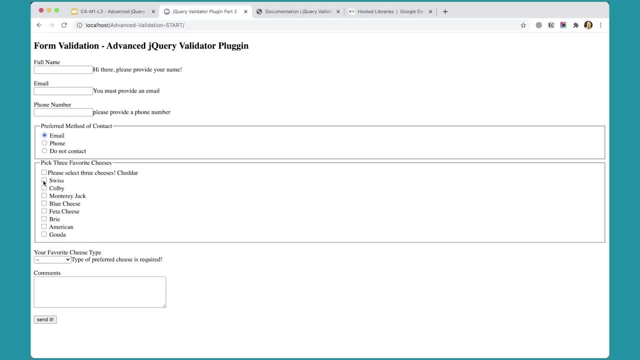 here it says: select three cheeses. notice, if I start checking these, once I've got to three, that message goes away and you could go from here and inspect these and see what classes are being attached to these messages and style them and do all of that right from here. but I want to show you one more. 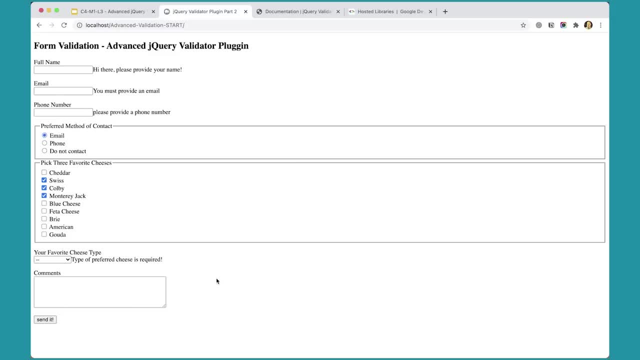 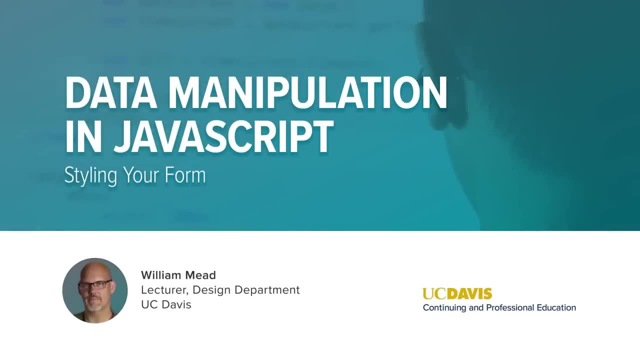 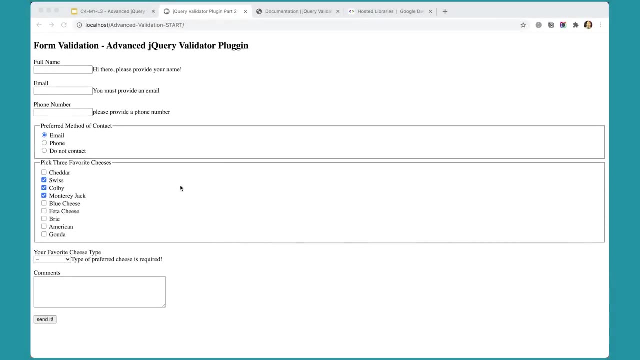 feature. that I think is kind of neat for this particular plug-in and we'll do that in the next video. we've gotten our validator working and we're going to go ahead and go ahead and see if it's working, and and it's, it's working great, and we've got our 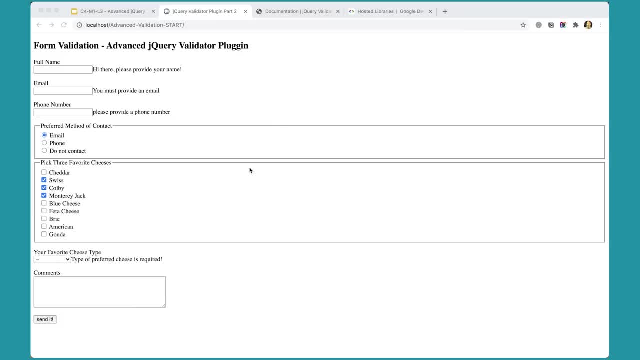 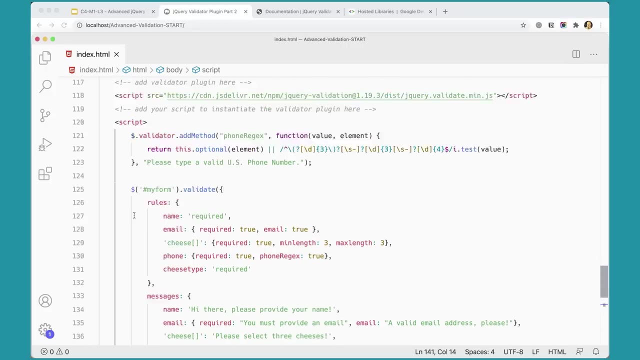 messages coming up. it just needs some styling. but what I want to do in this next feature is add a box over here and have all of the messages go into the box as as the errors occur. so let's go over to our code editor here and up here I. 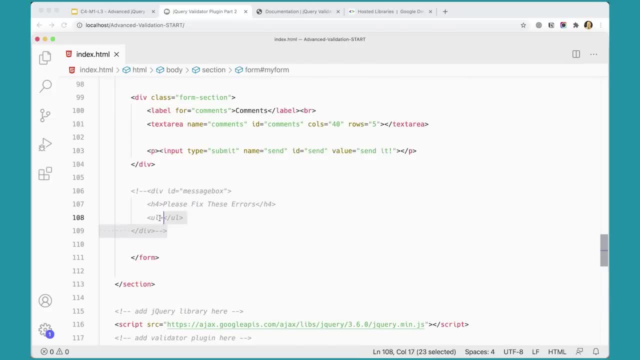 have this thing commented out, so let's uncomment this. so we've got div ID message box and then I've got just a low level header here- probably shouldn't be an h4, but that's okay- and an empty unordered list and we're going to add: 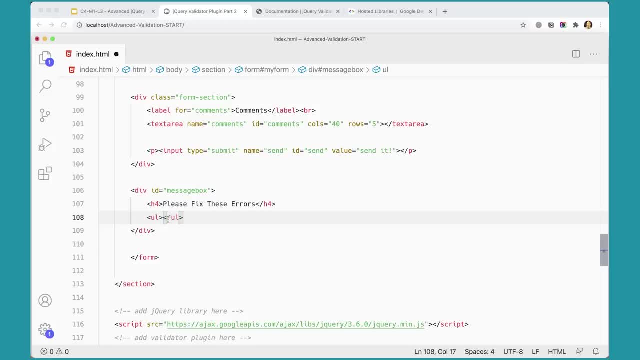 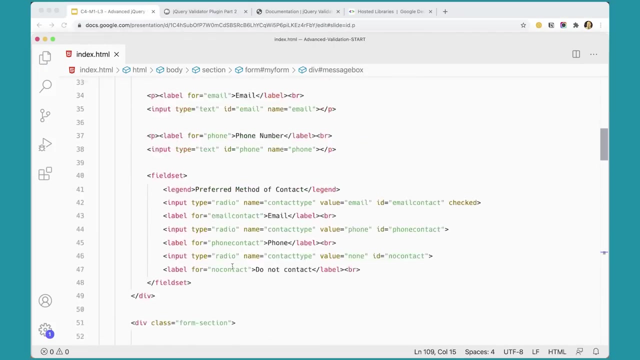 list items into this unordered list for each error that occurs. so let's go ahead and see how we can do that in our script, because I think that's pretty neat. oh, also, while I'm at it, up here at the top of the page, I have a little bit of 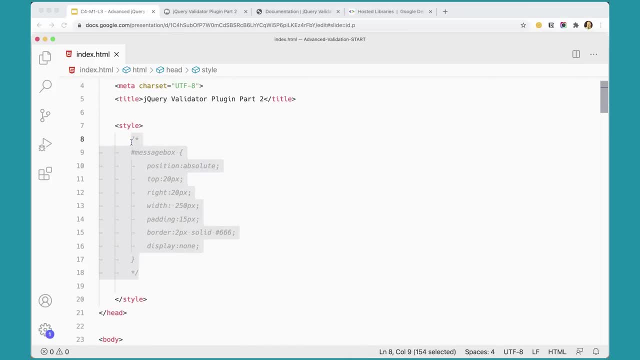 CSS here that I'm going to uncomment and that'll just place this, just going to position this box. we don't have a lot of nice styling going on in this form, but you could certainly do a lot more to make it look better. but I'm just going. 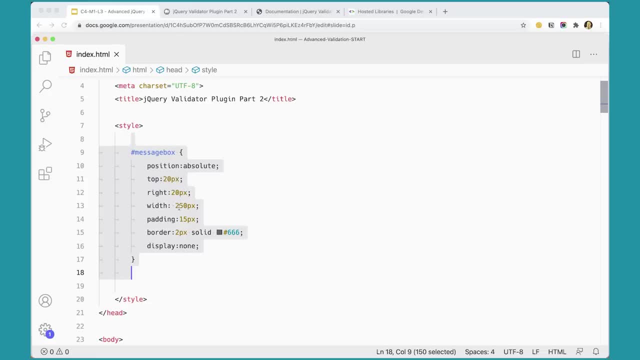 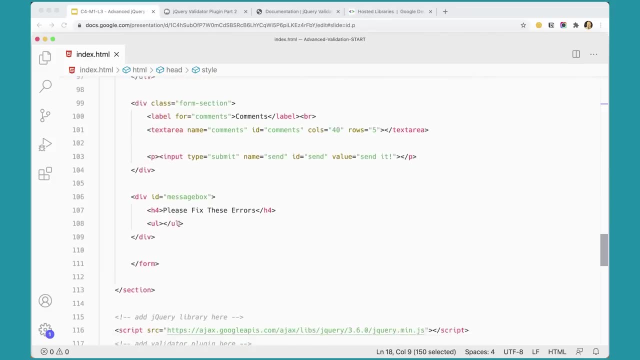 to position this, so this box, so it shows up on the side of the page over here. okay, now we're ready to continue to add to our script down here to see what we can do to make use of these, this feature here. so down here after message. 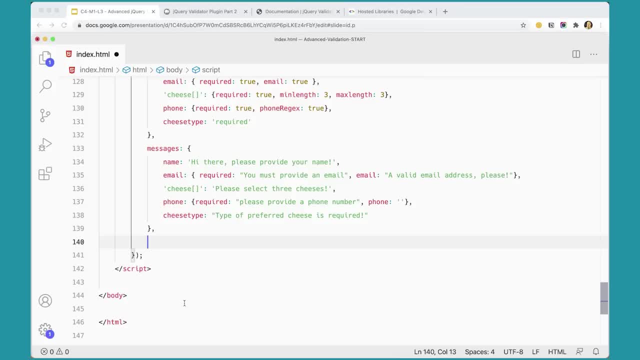 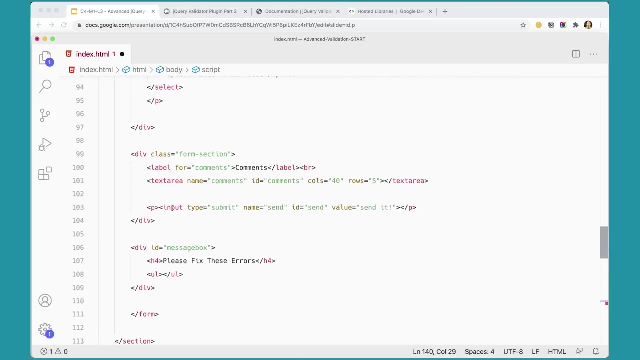 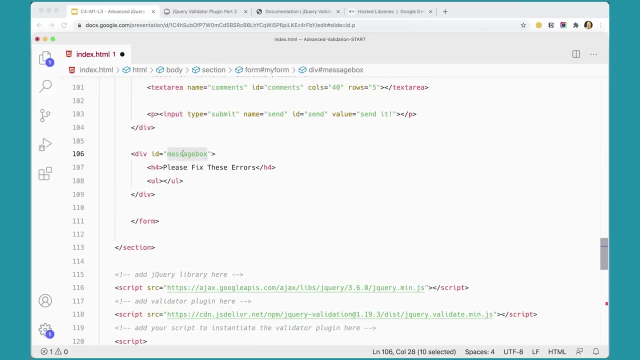 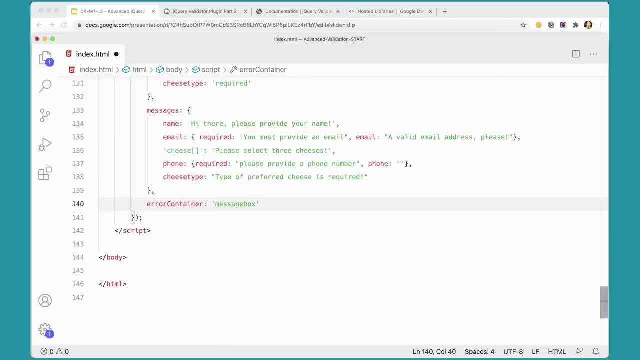 is I'm going to put another comma and then add a property called error container and that's going to be the ID of this box up here that I created where to go message box. this thing here, error container message box. it actually just pasted in there comma and then we've got it: error label. 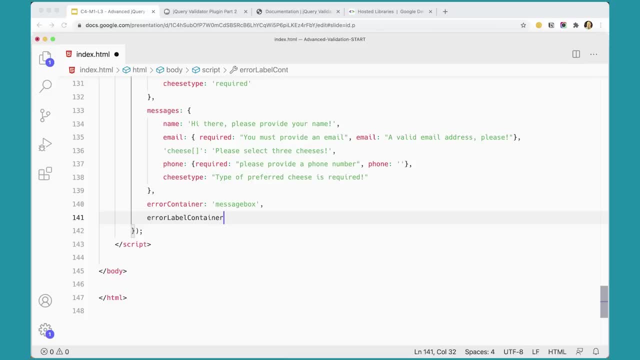 container and that's going to be. I'm realizing I forgot to put the pounds in here. don't forget the bandsite pound set. not going to forget to set what is the handset to do that. so that's the same thing, right to the path that I am as well. so hyperlinkcom. from this: insert those words that we are going to use down the right hand side and get rid of those symbols that we don't want. so coloring at the top of the page here the word error container without a��� and the data top donc to add those 코�. thus didn't work for many of the которые. 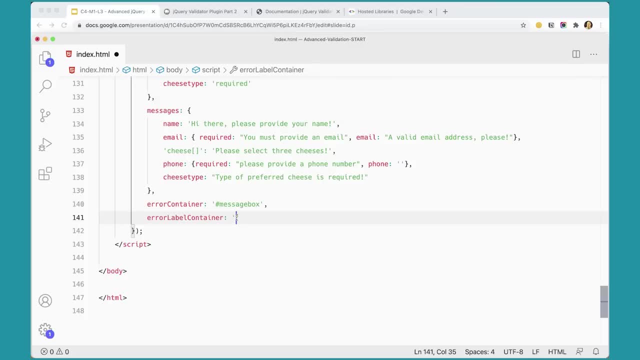 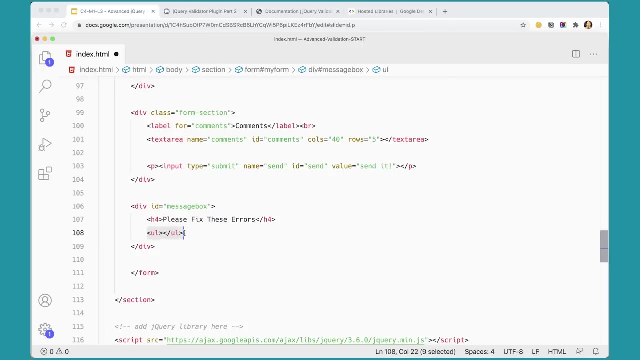 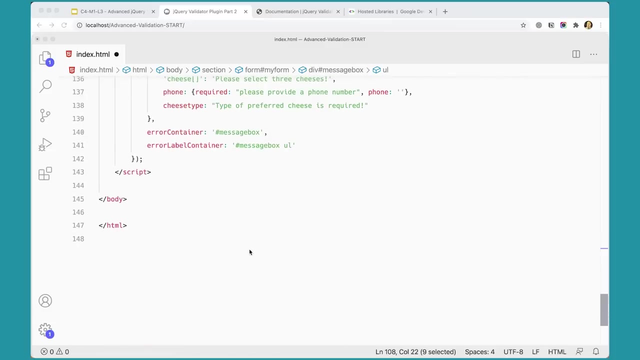 message box and this is going to be pound message box ul, because that's the error label container, which is this unordered list. here it's going to put the label. that's the container that's going to hold the actual labels. the put a comma here. the wrapper for the container is going to be list items like 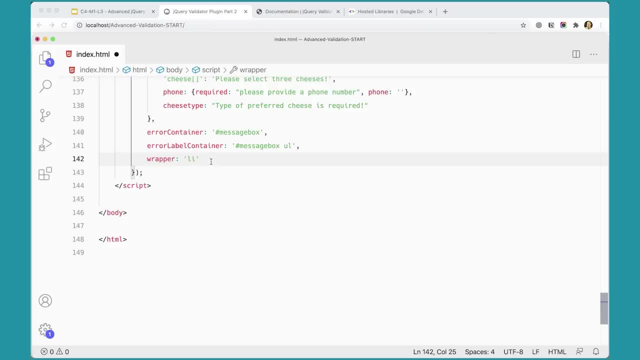 that again. how did I figure this out? working with the documentation on the validator plug-in website? you know I poking around in there's like oh, that'd be kind of a neat thing to do and it's really not that difficult to figure out. I spent an evening with it. I think it's pretty cool what you can. 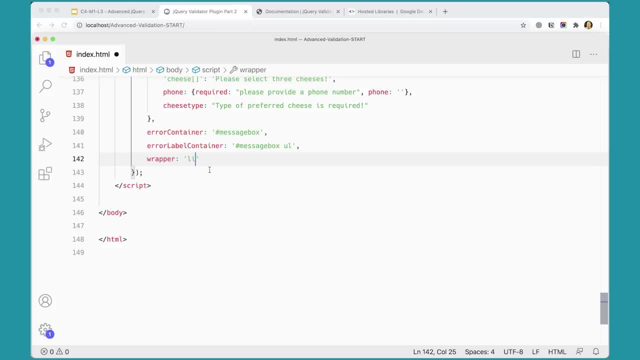 do with it. I think it's pretty cool what you can do with it. I think it's pretty cool what you can do with it. I'm just showing you the tip of the iceberg. there's tons, you tons more you could do with this plug-in. let's try it out, save the file, make sure everything's saved and then come back. 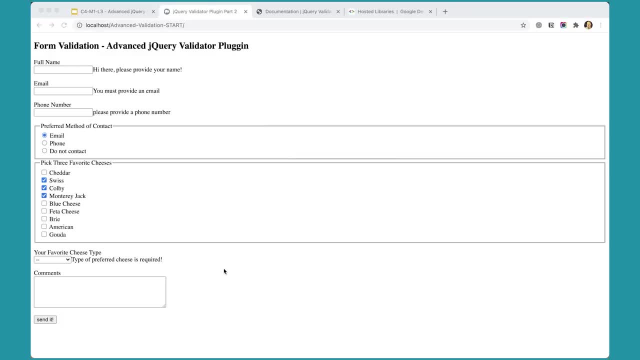 and let's try it again over here. so here I am on the website. on the web page, if I click send it, I should click refresh, send it. now I'm getting my error box over here. there'sion either tax slider or your configuration, which looks kind of funny. 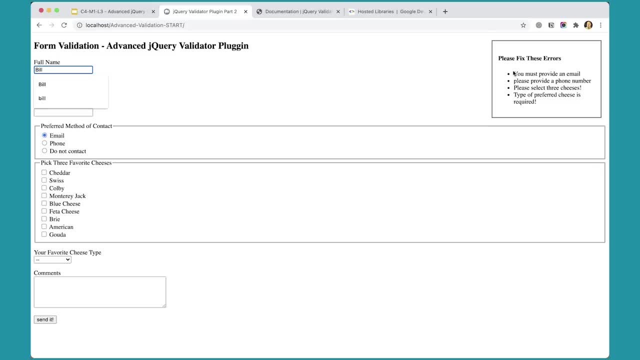 but that's okay. but it's showing my errors over here and you, as you fill this out, bill notice: the error for the name went away. if I put it in something that's not an email address, it'll say a valid email address. please, yeah, somewhere com. 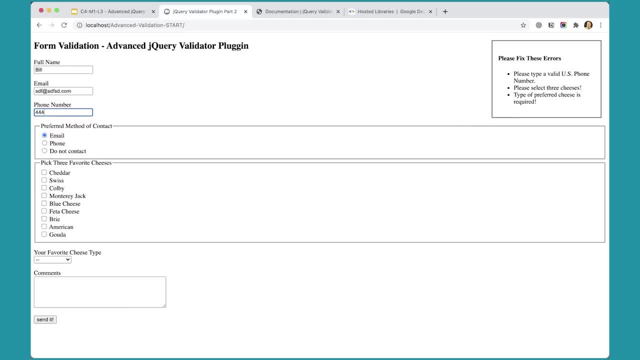 I can do some random phone number and it's going to want a notice. it's saying: type: a valid US phone number now preferred method of contact when it is selected down here. I have to pick three cheeses. so I pick one, two, three and that message goes away. 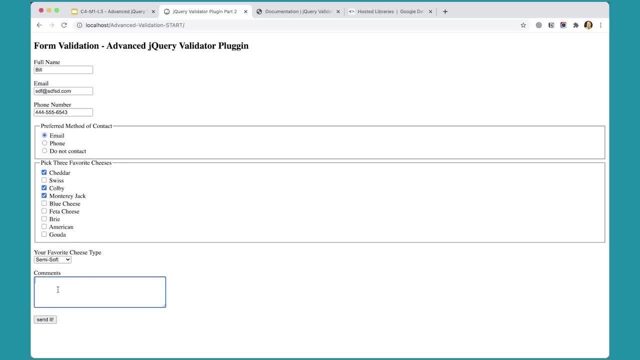 I have to choose something from here, add some comments, hello, and when I click send it, I get my process data because I'm running this on my local host, so it's coming through. If you've got a bunch of PHP here, that's fine. it's just because you're running it locally, but the processor is actually working. 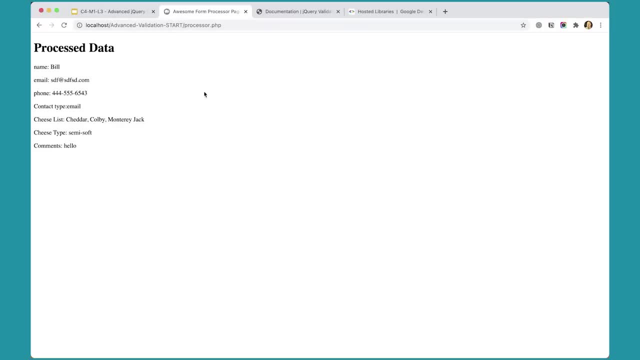 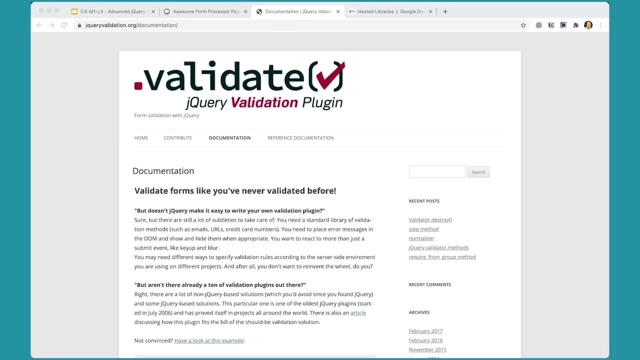 So this is a really great little project that will help us, a great plugin that will help us Make our forms more accessible and easy for users to use, and that's a really important thing to be able to do. I recommend poking around on the plugin on the validate plugin website so you can see what else this plugin can do. 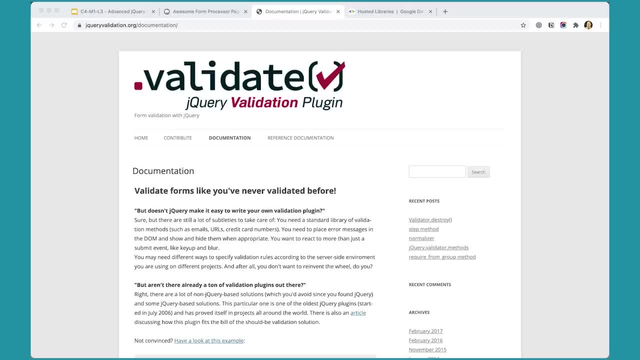 There's all kinds of really interesting things you can do, and I recommend playing around with some of the features. If you don't want to use jQuery and you want to try a different library, there are lots of libraries out there specifically for validating forms. 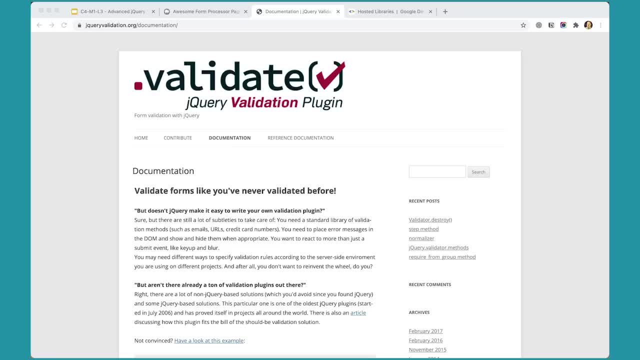 You know, it would be kind of interesting to compare some of the features of some of the different libraries. So if you just Google or search for different form validation libraries, you'll find some out there and you can try them with your forms and see how they work. look through the documentation. 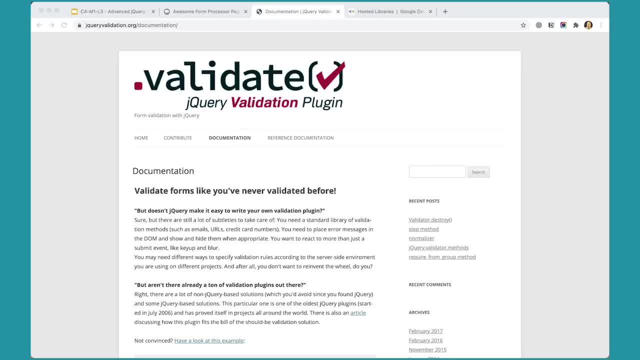 It's a really great way to learn JavaScript and to learn how to use some different tools that could be handy for a lot of different purposes. It's a really great way to learn JavaScript and to learn how to use some different forms that could be handy for a lot of different purposes. 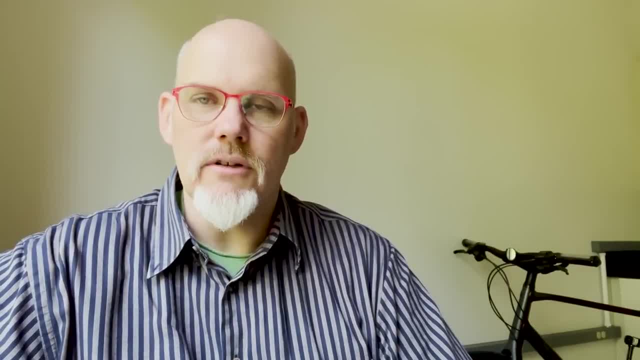 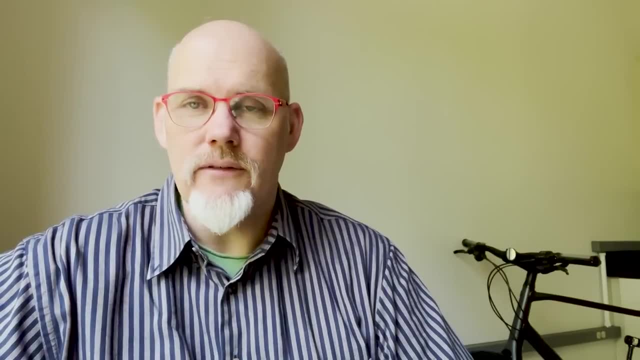 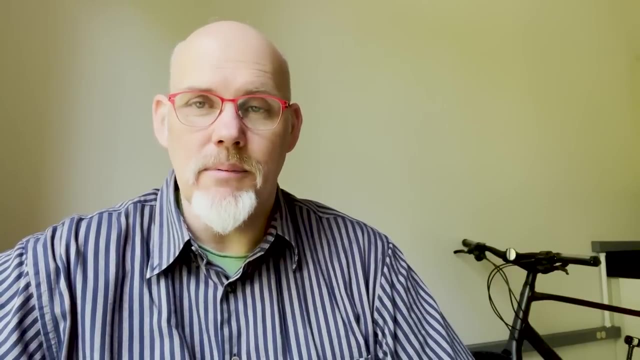 Hello and welcome to our second module in our fourth course on JavaScript. In this module, we'll look at prototypical inheritance, which is a fantastic and powerful feature of JavaScript that's frequently misunderstood. With a strong understanding of how prototypical inheritance works, you'll really be able to push your JavaScript skills to the next level. 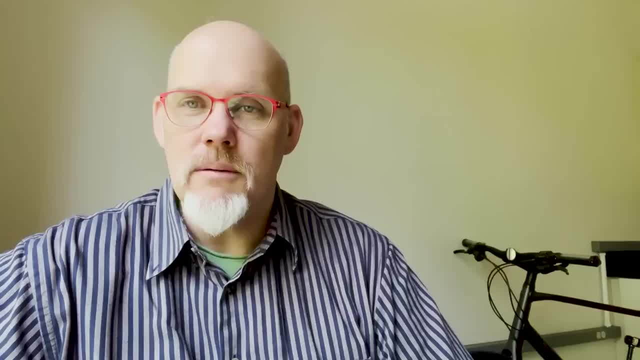 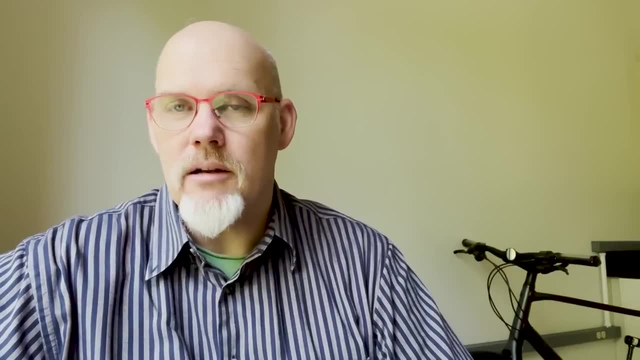 Plus, we'll start working on a project that we're going to complete in the third module of this course. I think you're going to get a lot out of the planning process and it'll really help you learn how to plan a more complex script. 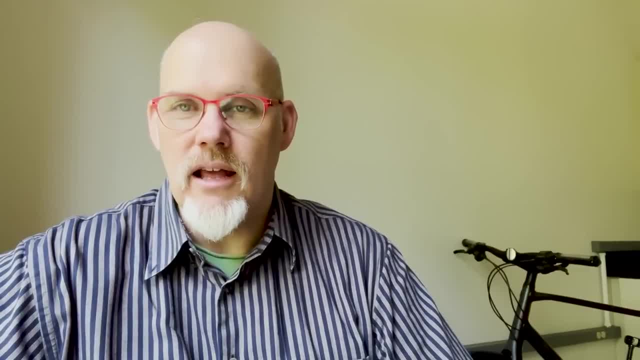 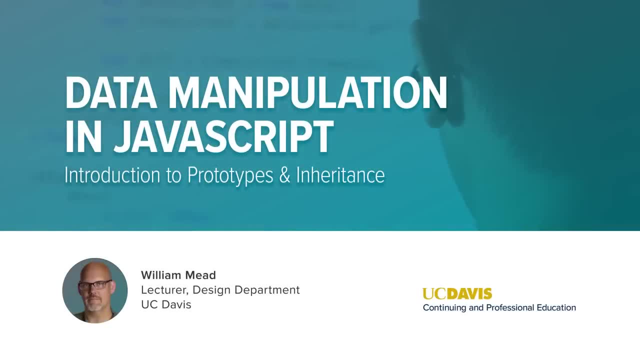 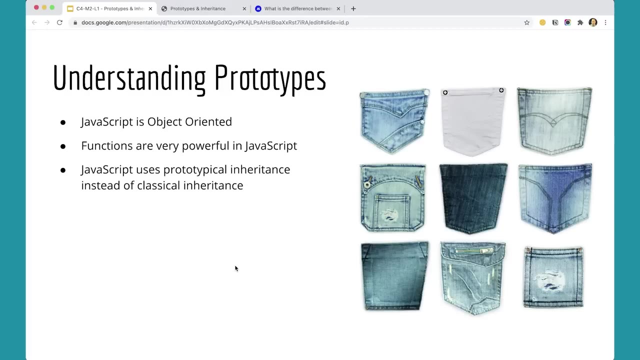 So let's dive in and get going on this. I think you're going to get a lot out of it. Prototypes and Inheritance. It's a common misunderstanding that JavaScript is not object-oriented. It is object-oriented. It's true that it doesn't work with classes the way other languages that use classical inheritance work with classes. 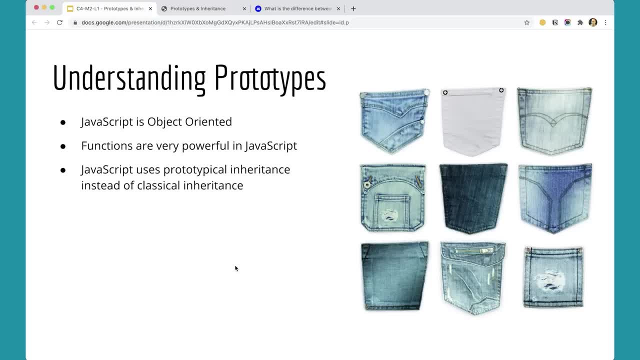 But JavaScript has what's called prototypical inheritance And the functions in JavaScript are very powerful And between the prototypical inheritance and the use of the functions in JavaScript you can mimic a lot of the functions in JavaScript. There's a lot of the same features that you can get in other languages that have classical inheritance. 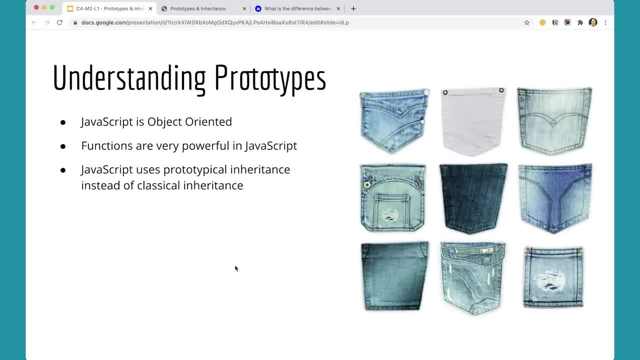 And you can do all of that in JavaScript and it's very powerful. Now JavaScript does have a class keyword now, but really that's just what we call syntactic sugar. that will make it easier to work with the prototypical inheritance. 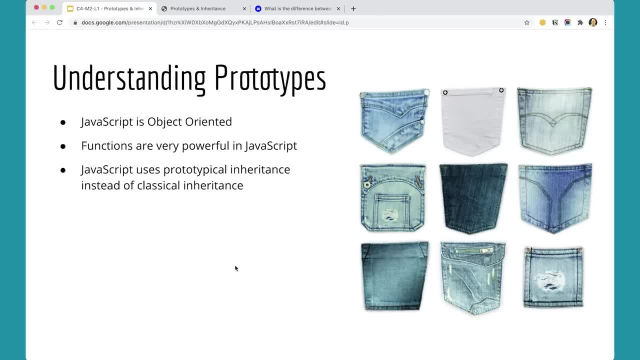 We're not going to use the class keyword in this course, but it's worth knowing that it's out there. I put on this in this video here, this picture of these different pockets, because I think it's a good representation of what classes could represent. 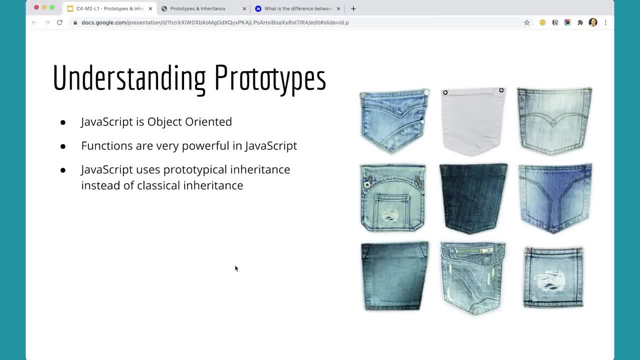 We have an object that is a pocket, but a pocket could look really different. It has some similar features in that you can put stuff in a pocket and that it has some common functionality, but it could have different features or look a little bit different in different places, in different scenarios. 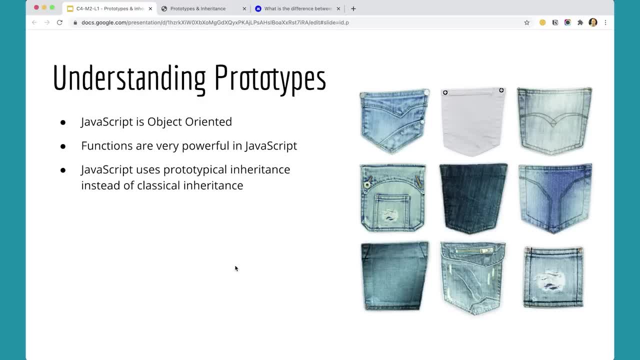 So I like that image there. This is a reminder of what a class could be, which is an object that has similar properties to another object or to a parent object, but then has its own unique properties as well. Let's look at an example where we can create a prototype. 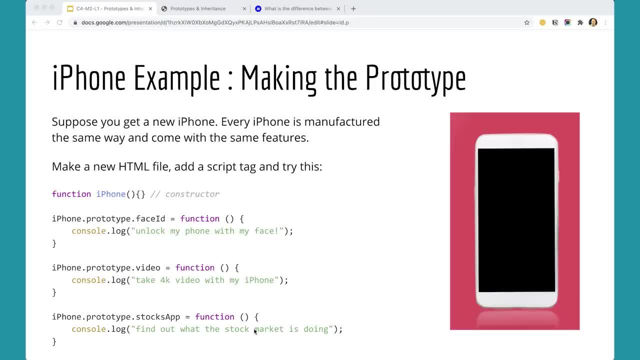 that then we can use as sort of a template to then make a new version that will inherit from that prototype, but the new version will have its own features, And we'll use the iPhone example here. And, by the way, I think it's worth giving credit to this article over here. 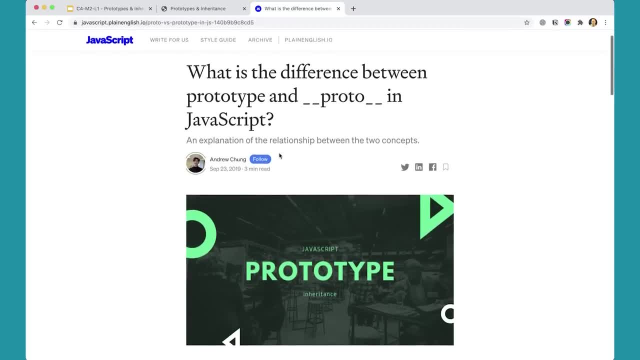 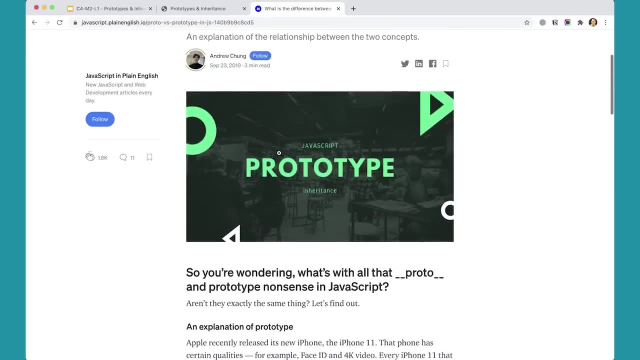 which I will provide a link to. It's a good article and worth reading in its own right, but sort of some of the ideas came out of this article, although I went my own direction with it, But I wanted to give credit to this author, Andrew Chung. 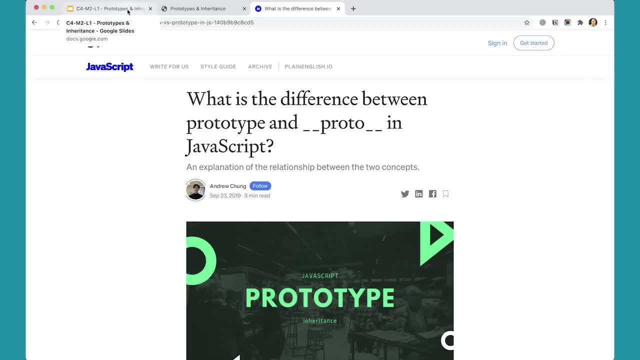 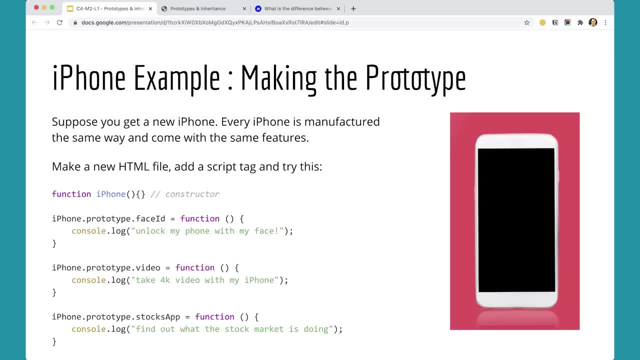 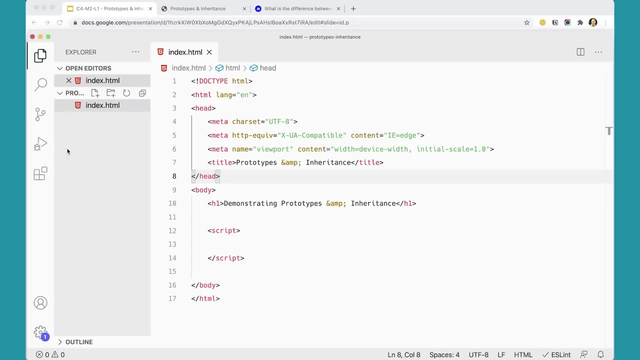 here for coming up with this idea, because I'm using it to explore and explain this here. So make a new HTML file. And over here I have a new HTML file And you're just going to add this script in here. So I have an HTML file that I've made. 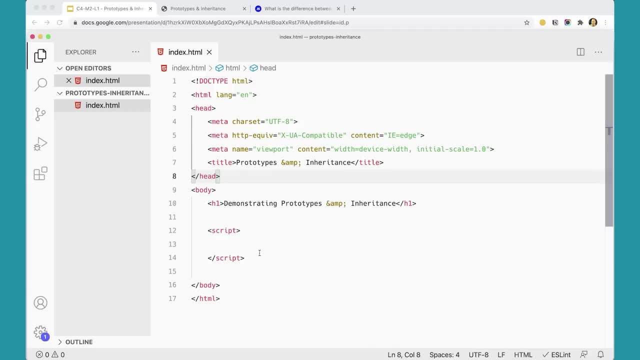 and I just have an h1 here demonstrating prototypes and inheritance And then I'm going to paste in here. The amp will produce an ampersand. I'm going to paste this content in here. That was the link to the article. Here's the content I'm going to paste in here. 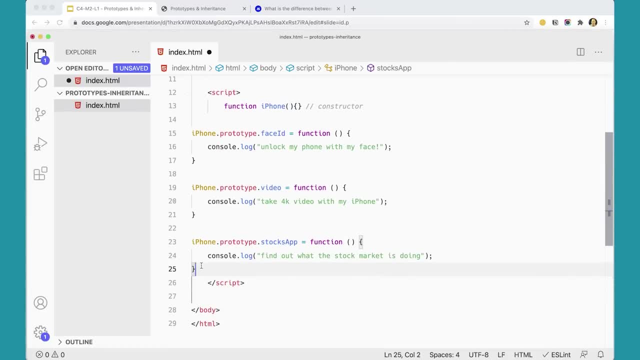 Okay, So I'm just going to tab that in properly, Folding that up there. Tab that in properly. You're going to have to type this, but I'm pasting it in. But I've created a function here called iPhone and it's a constructor. 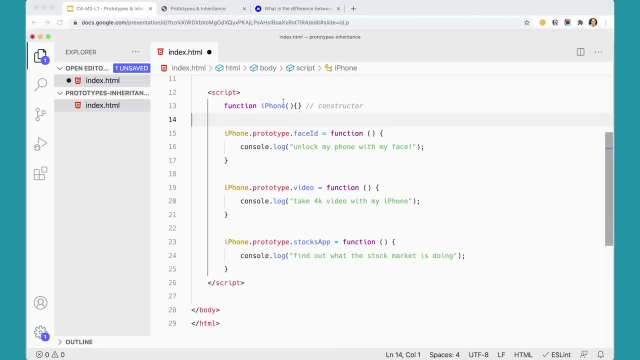 It's basically an empty object here, that's just got nothing in it. And then I'm adding things in using this prototype keyword that adds these features into this object, into the iPhone object here, And it's got face ID And this holds a function. 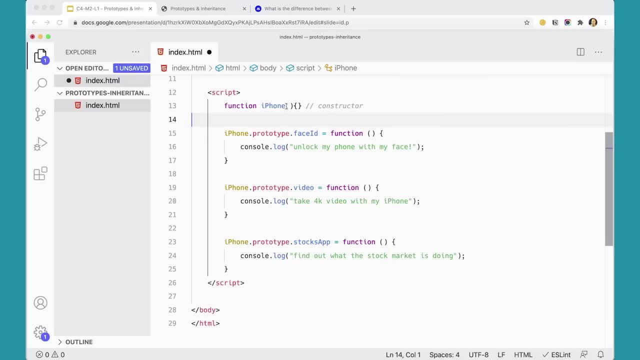 So it's a method, because this is a function that belongs to the object. So we call that a method And this method. all it does is console logout, Unlock my phone with my face, So that's a feature that belongs to all iPhones. 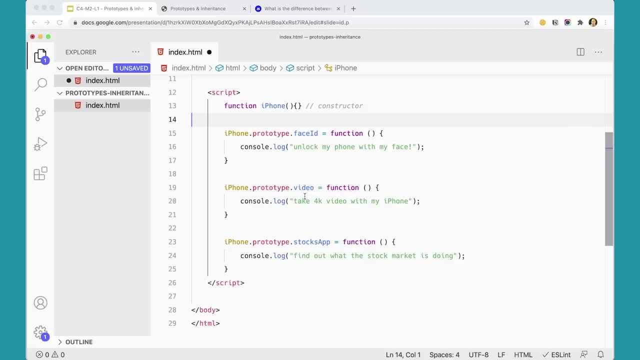 It also has a feature called video, which allows me to take 4K video with my phone. That's a feature that all iPhones have. And then I have another feature, which is the stocks app, which is a default app that comes on every iPhone. 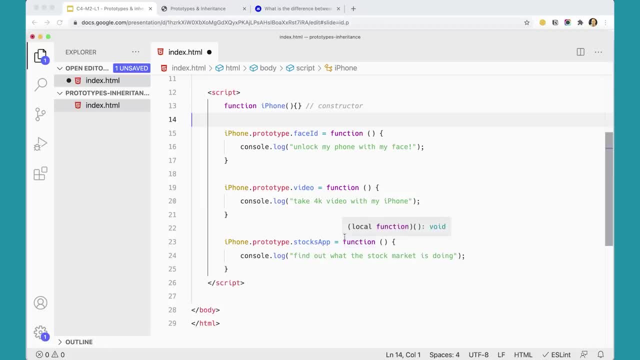 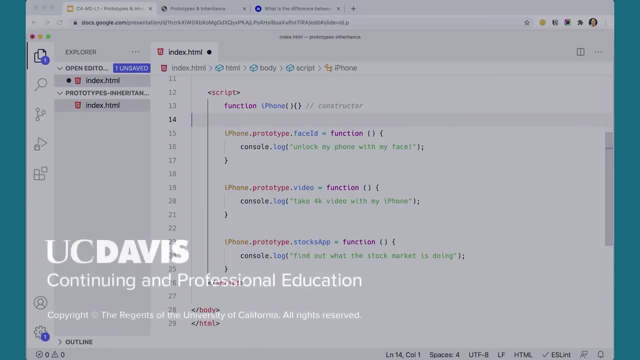 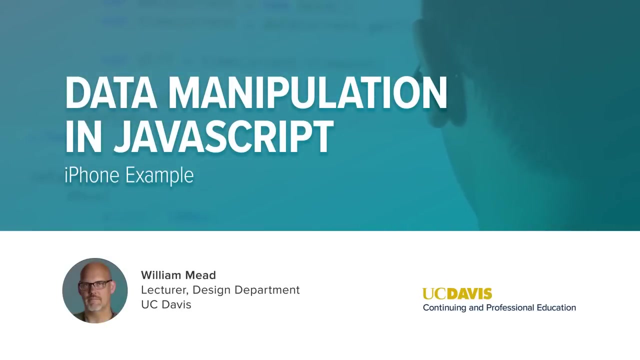 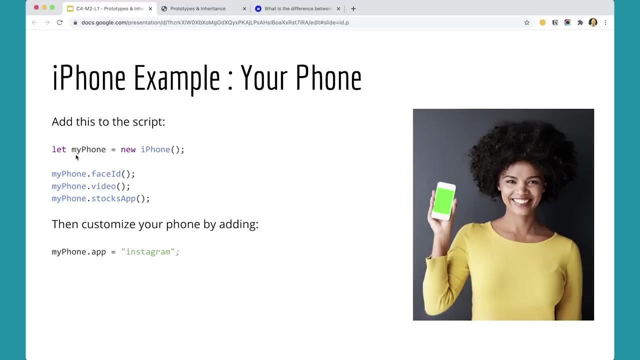 that will allow you to find out what the stock market is doing, And we can continue to add additional features into this prototype that every iPhone might have in it. Now you can add to the script a. we're going to create an object called my phone. 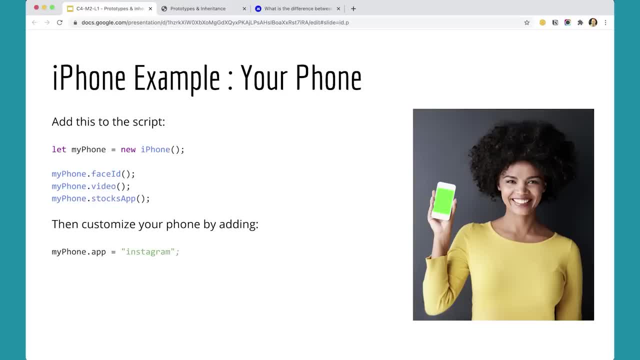 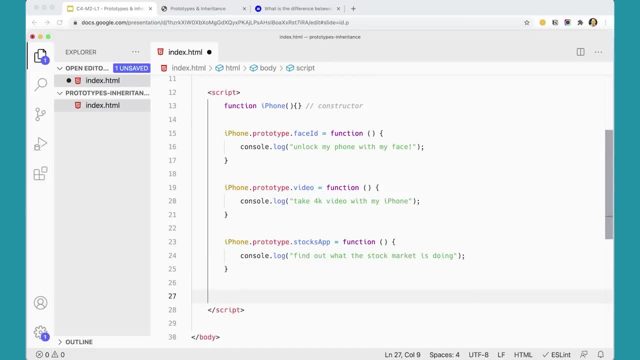 which is going to be a new iPhone, So we can add that to our script over here- Let my phone- and that's going to be assigned a new iPhone. So now my phone is going to inherit all of the features that iPhone has. 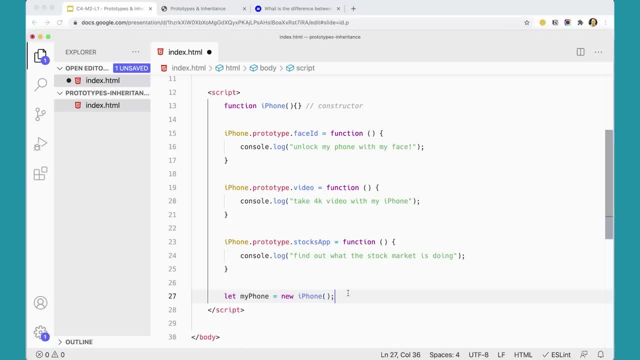 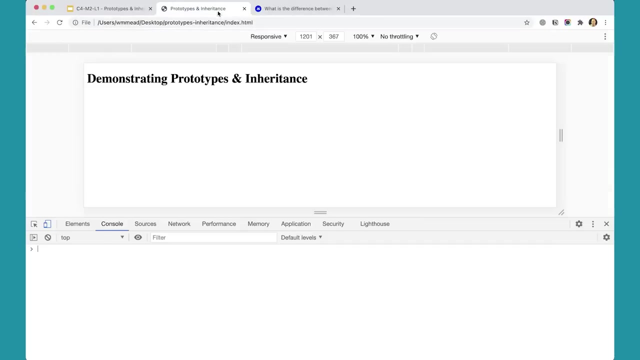 that every iPhone has, because my phone comes. it's an iPhone, so it comes with all those features, So I can do things like my phone dot face ID And you'll see. I have this file up and running over here And if I come back and refresh this, 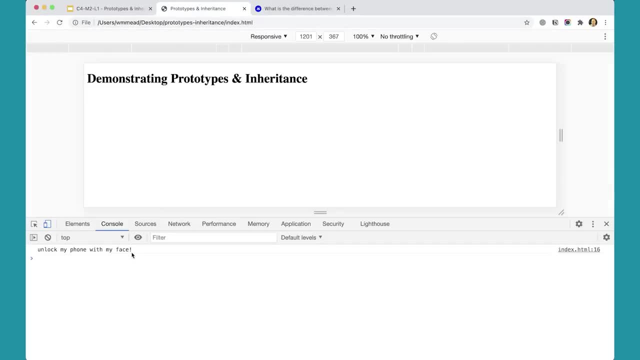 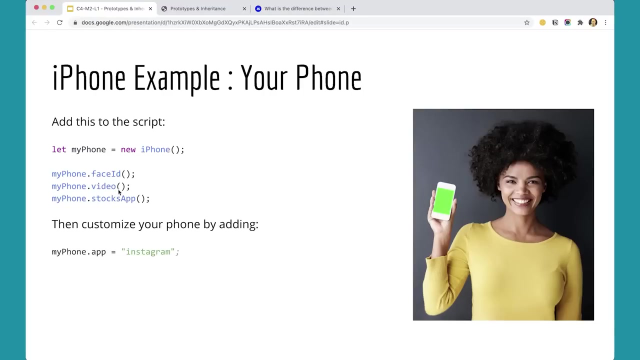 I can unlock my phone with my face because it now it inherits that feature from from the iPhone prototype, And I can do the other features as well. So we come back here and we could add my phone video and my phone stocks app. 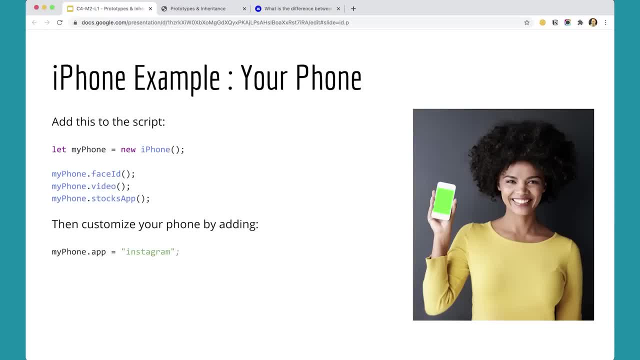 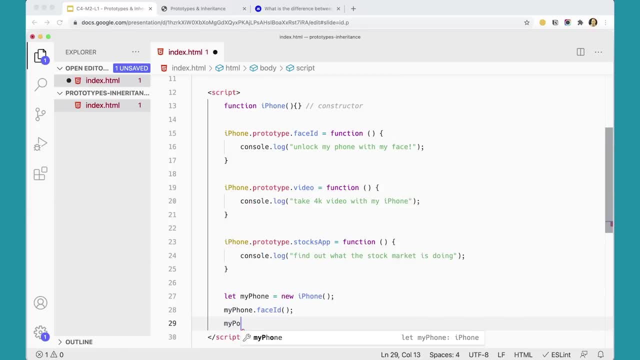 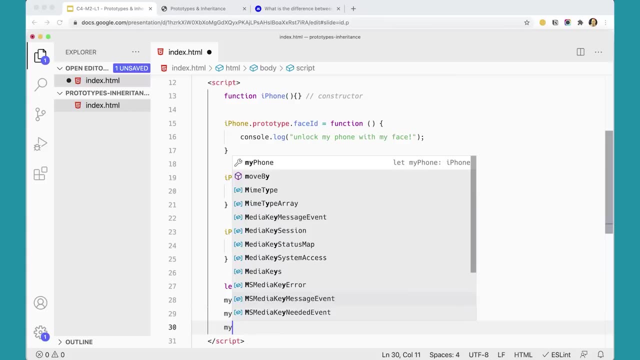 and you'll see that it actually does that, That it actually does those things as well. My phone dot video spell phone right. My phone dot stocks app And you'll see, if I save that and come back and refresh the page, that my phone has those features as well. 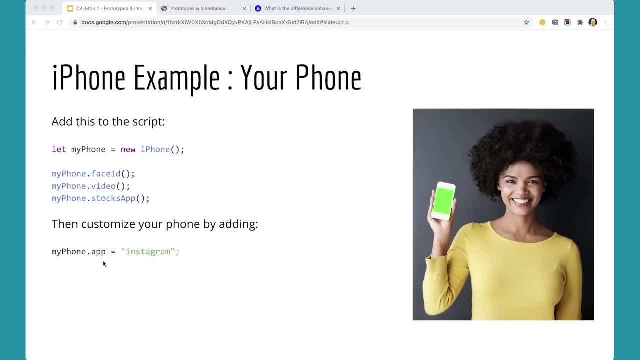 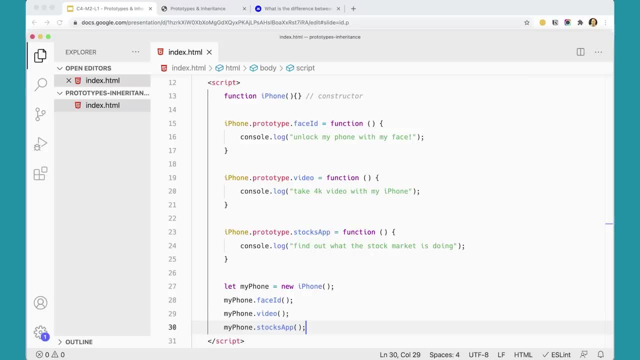 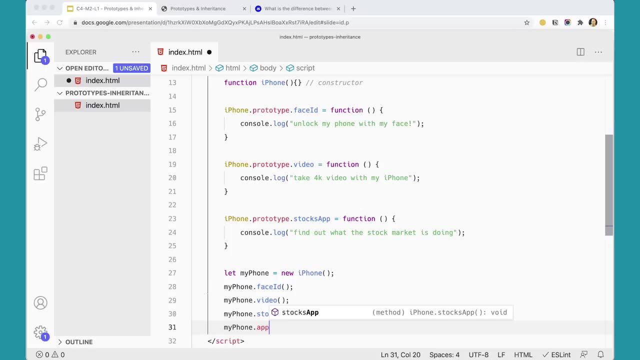 We can further customize my phone by adding an app So you can go to the app store and download an app. Suppose I add Instagram, So let's go ahead and add that My phone dot app equals Instagram. And now if I were to do my phone dot app? 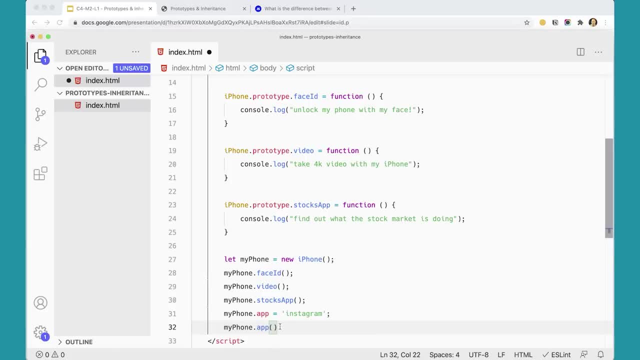 Actually, let's wait on that. Instead, I'm going to do console log my phone. So I didn't make the my phone Instagram app actually do anything, So I'm going to just console log my phone here and see what I get. 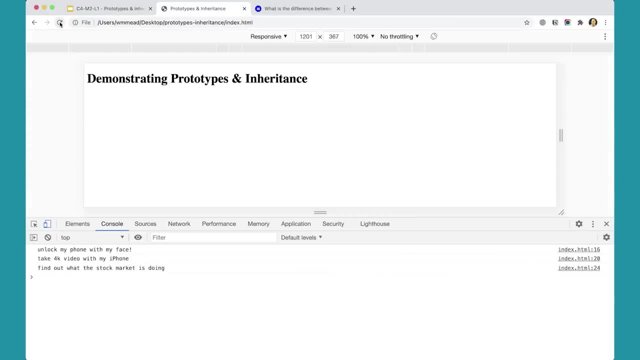 So if I come back here and refresh this, you can see I can still unlock the phone with my face. I can take 4K video, I can find out about the stock market and how that's doing. But then my phone: it has an app: Instagram. 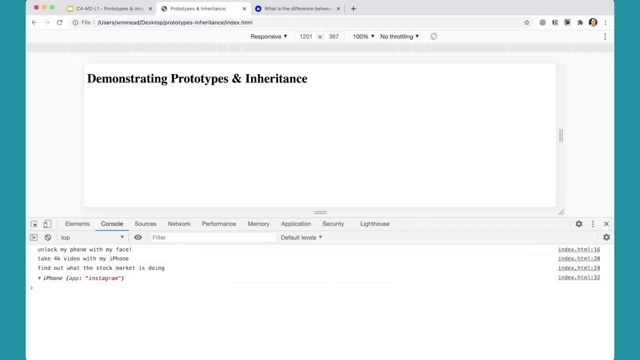 It's showing that this app is on here. Furthermore, if I toggle this little arrow down, you'll see: okay, we've got our Instagram app, And then you see this thing: underscore, underscore, proto, underscore, underscore object. And that's because this thing is inheriting from an object. 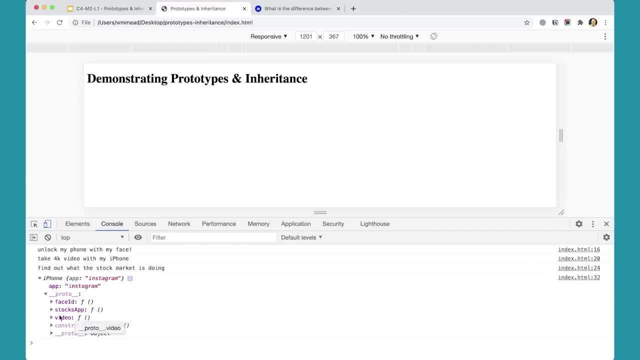 And it's got. you can see here the face ID, the stocks app and the video And then down here underscore, underscore, proto underscore, underscore. object again, because in general in JavaScript, many of the items in JavaScript are ultimately objects that inherit from the object. 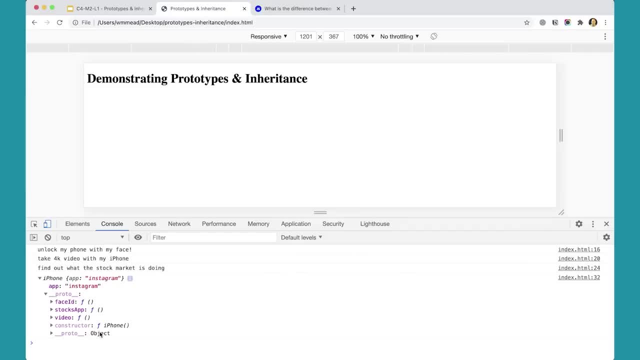 the object object, essentially in JavaScript. So we can follow everything back all the way back to this object thing in JavaScript because it's an object. You could fold this down to see all the properties that objects, objects, have, as in JavaScript. So it's a constructor for an object. 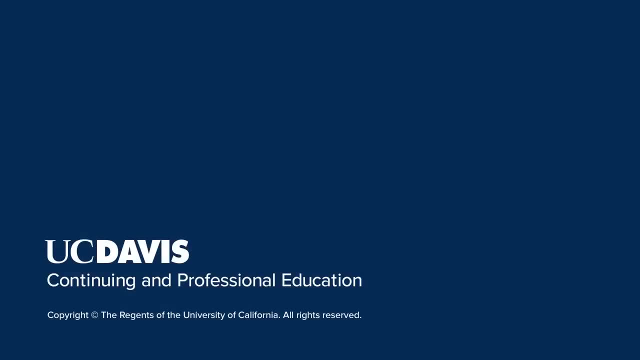 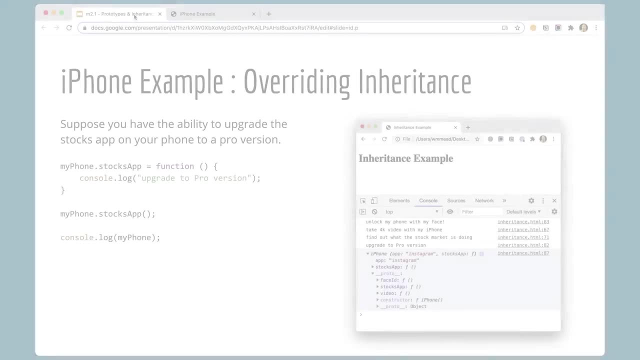 It has a property, all this stuff. One important feature of prototypal inheritance is that you can override it. So, for example, I could take my iPhone stocks app and override that app with a pro version. So let's go ahead and do that. 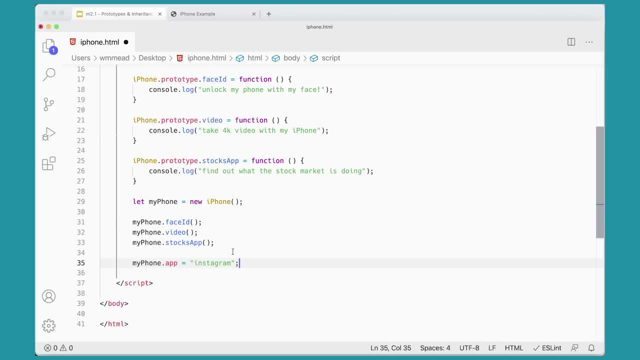 I switch over to my code editor over here. I can come down here and add my phone stocks app and that's going to be upgrade to the pro version here in the console log. So that's all that's going to show here. But now, if I do, 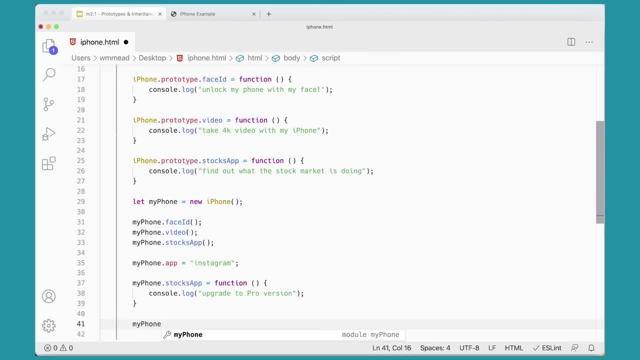 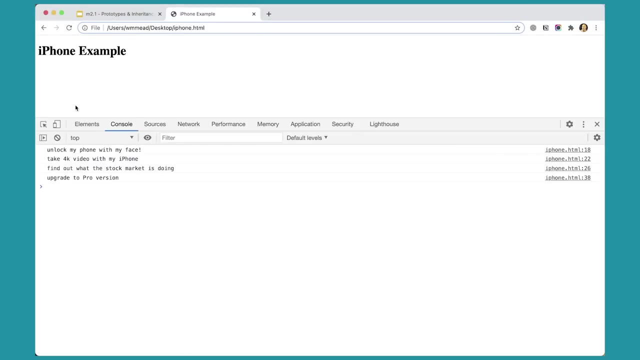 my phone dot stocks app, like so, and then run this over here, you'll see upgrade to the pro version here. But also now if I come in here and type my phone again, you'll see it's got Instagram plus, it's got the stocks app here. 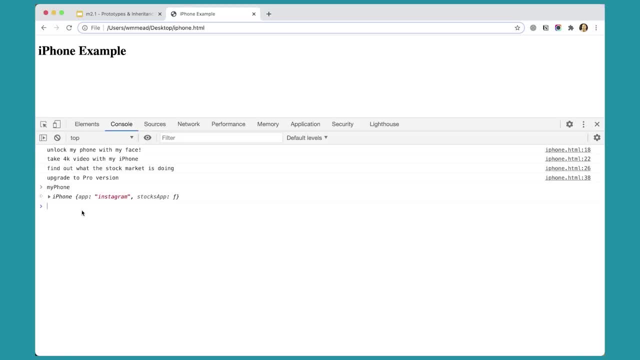 that's been upgraded. That's a function And if I go down here but you'll see that it's still inherited the stocks app. It's just upgraded it, So it'll use this one, but it still inherits the stocks app from the prototype. 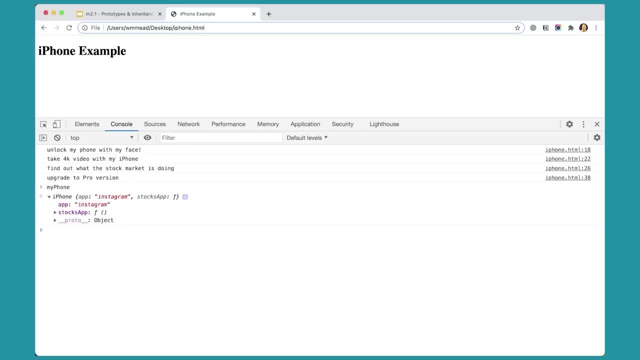 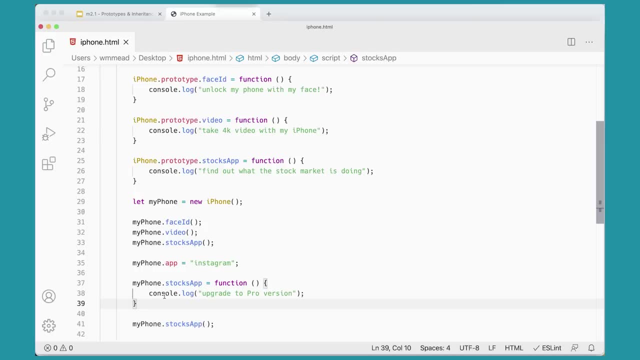 which is interesting. Or suppose we don't? we don't want the stocks app at all, For whatever reason. we decided we want to delete it. We could do my phone stocks app equals undefined And that basically leaves it as an undefined variable. 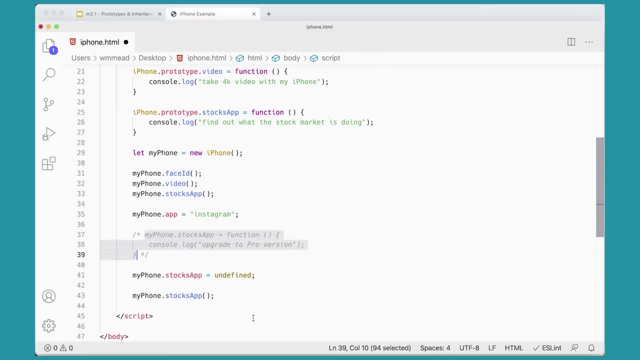 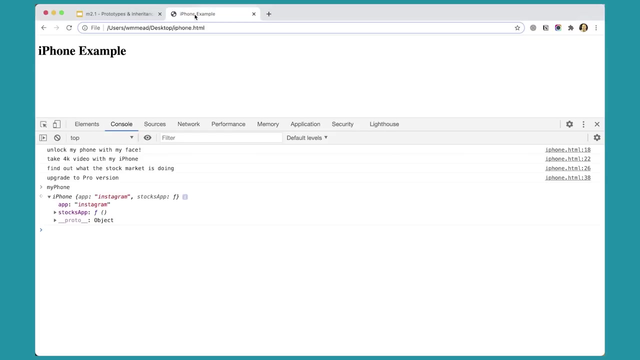 I'm going to comment that one out And down. here I can just do console dot, log my phone And we'll see that it's not in there anymore. Come back and refresh this. So I've got my phone and then stocks app undefined. 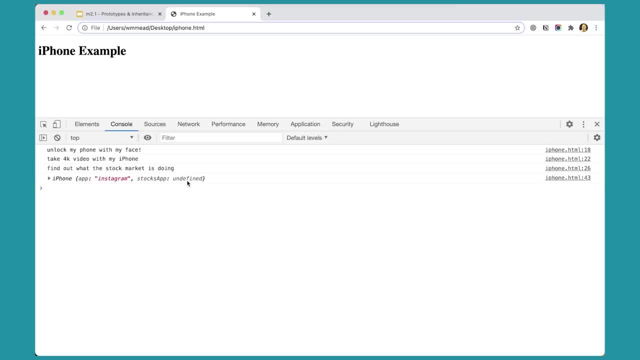 It's no longer a function And you could actually delete it with the delete method, But I wanted to show that you can leave it as undefined. but it is still inheriting the stocks app from the prototype here. Here it is there. It's inheriting that function. 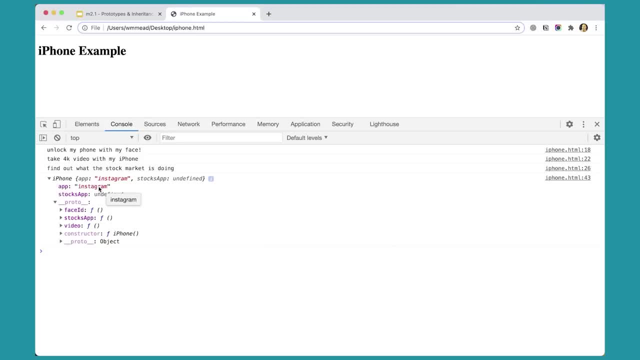 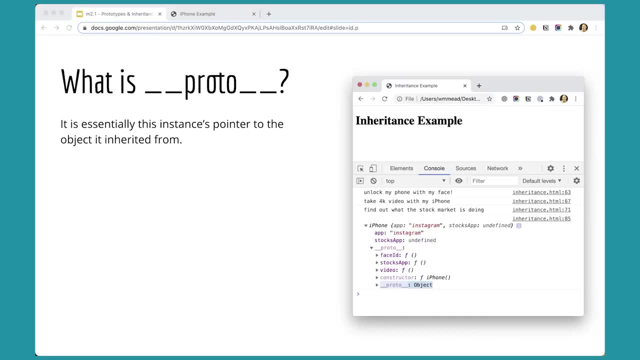 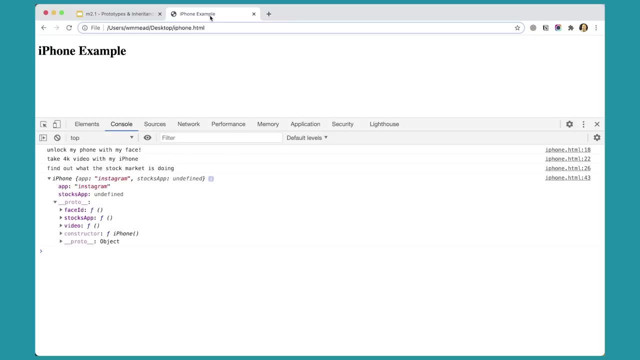 We've just sort of undefined it And left it so that you can't use it anymore. What is proto? Proto is essentially the instance's pointer to the object it inherited from. So as we look in here, we can see under proto: 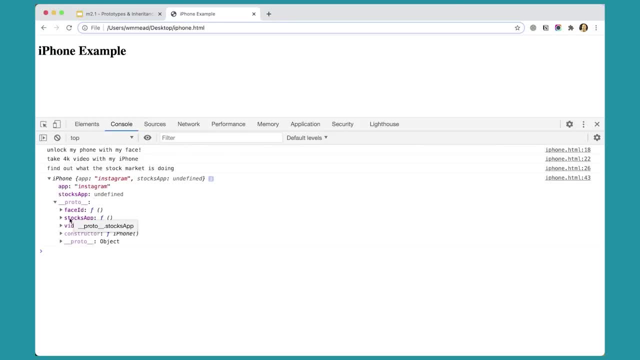 that's the object that it's inheriting from, And then down here we can see object. Now this is worth doing as well If we go into our page here and just make for a moment, just make just a basic array. 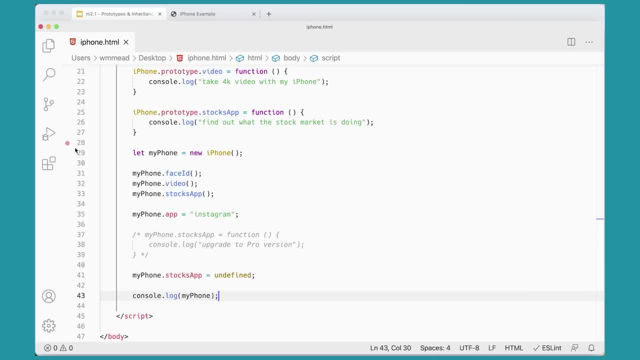 just like we did in the very early parts of the first course in the specialization. If I come in here and say, var my animals equals square bracket, chicken, dog, turtle, llama, whatever it is there, we can go ahead and add some animals. And then, if I do, 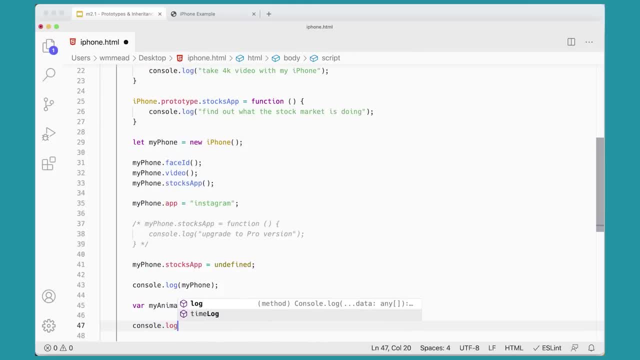 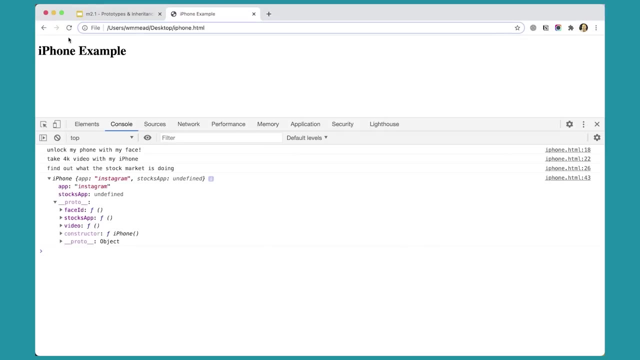 console log animals, my animals. there we go And then come back here and refresh this page. You'll see we get the array. but if I toggle this thing down, there's the elements in the array. It gives me the length property. 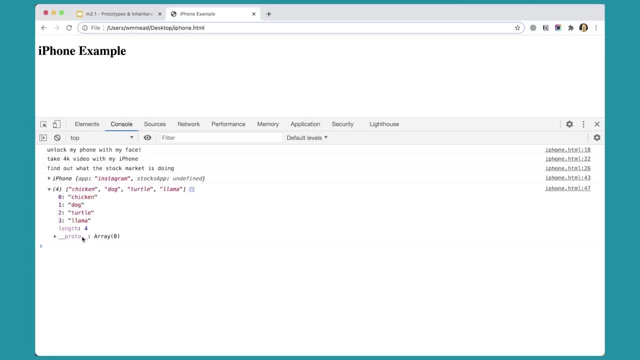 which is four. And then it says proto array. So this instance of this array is inheriting from the array object. And if we go into the array object we'll notice that there are a whole bunch of array methods And we've been using those methods. 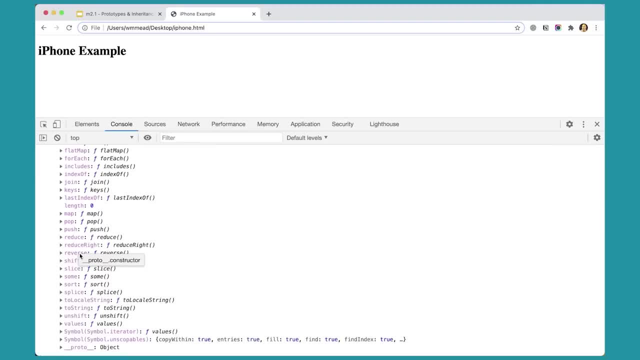 since the very early part of this course. There's all kinds of methods that we can use, like push, for example, to add something to an array or splice or index of. There's lots of different methods, And those methods we call them methods. 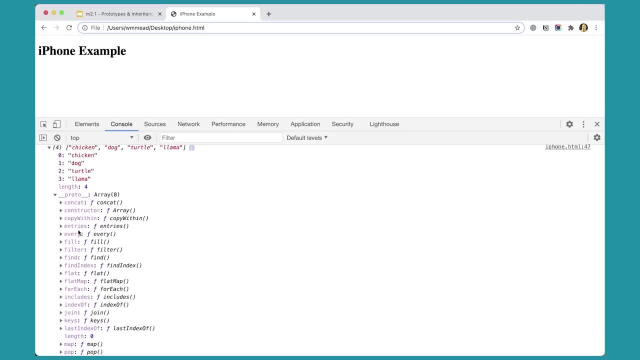 because they belong to the array prototype object, So that anytime you make an array you're creating an instance of the array object and you have access to all of the methods in that array object. So we've circled around to the beginning of this course. 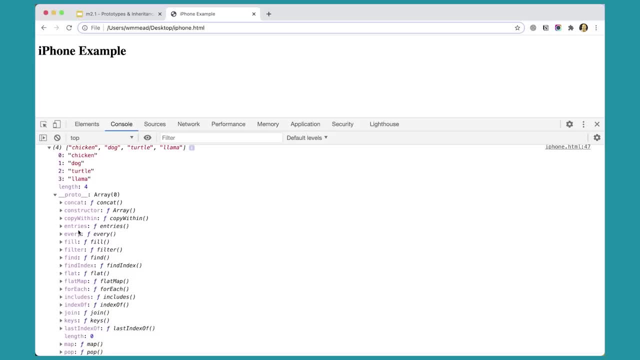 in a way that's really important to understand because it has everything to do with the way JavaScript works with prototypes and the way in which it's object oriented. If we dig in further, after the, the array object, it also inherits from the object object. 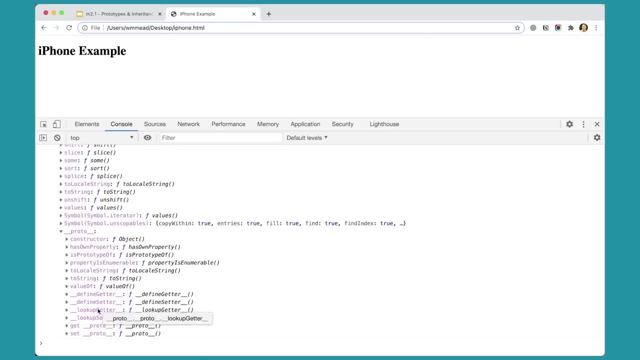 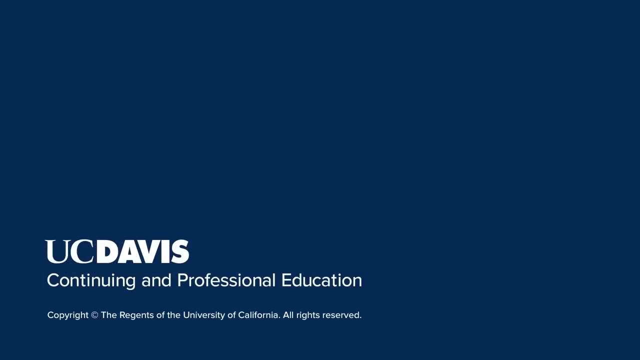 which has its own set of constructors and set of methods and properties. And so every time you're making an array, you're making an instance of the array object, which is really an instance of the object object. Hopefully that makes sense. Let's take a look. 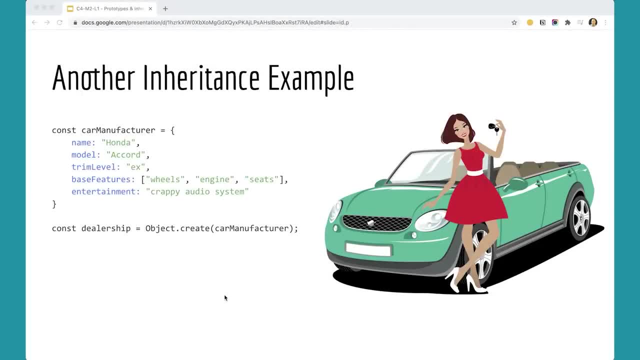 at another inheritance example. really to just drive the point home, no pun intended, But suppose we had a variable called car manufacturer and that variable's going to hold an object And the object describes some features that a car manufacturer might build into a car. 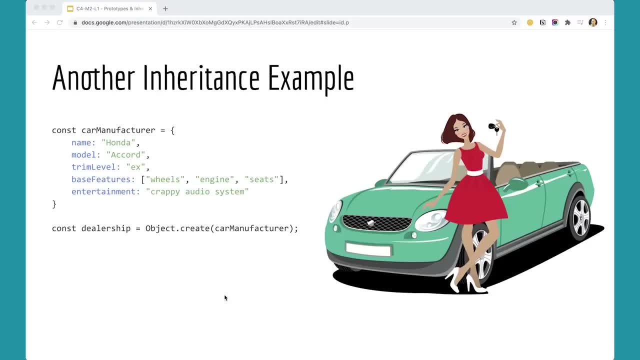 So they might have things like the name of the manufacturer, the model of the car, the trim level, some base features perhaps- And you'll notice that that's holding an array of features- and perhaps some other features like an entertainment system or something like that. 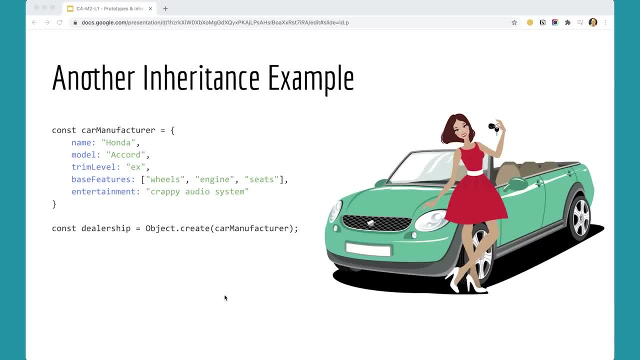 And then suppose you create a variable called dealership And the dealership is going to be assigned object: create car manufacturer. So now the dealership variable holds in it all of the things that the car manufacturer holds in it, Because when the dealer gets the car 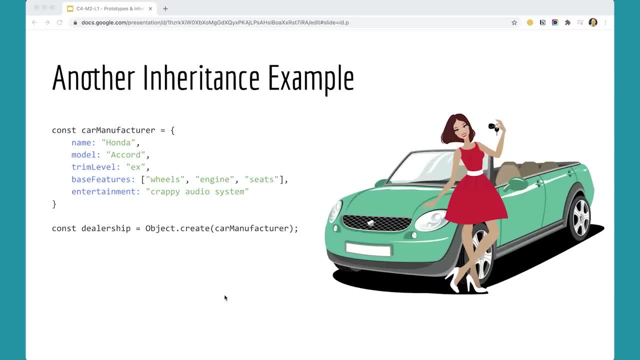 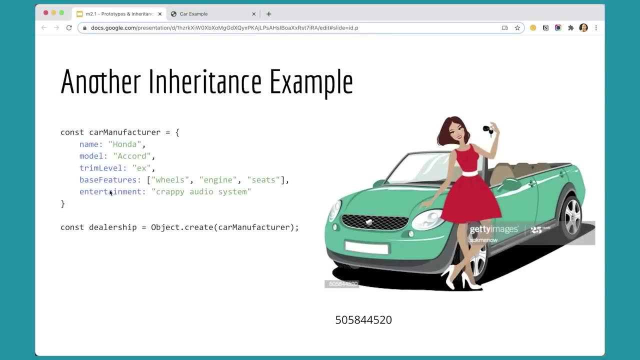 they get it from the car manufacturer and it comes with those features, And then the dealer might add their own features on top of that to the car. Let's go over to our code editor So we can create this object here, And then we're going to create. 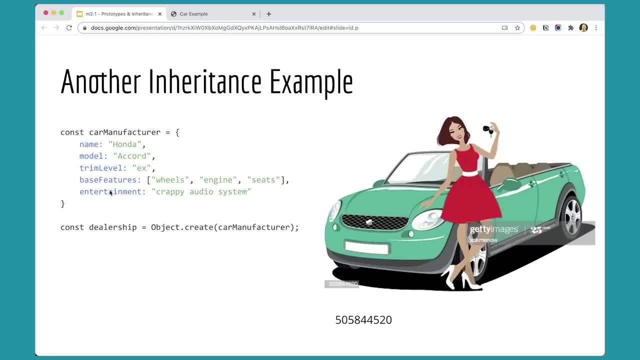 a new instance of that object by making a, a variable called dealership, and using object create car manufacturer will mean the dealership will have everything in it that car manufacturer has in it. So the dealership gets the cars from the manufacturer and they come with things like: 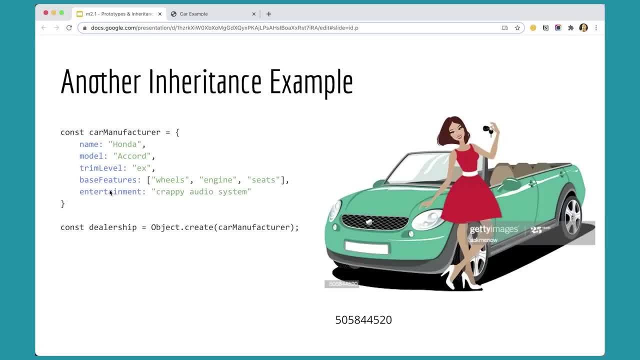 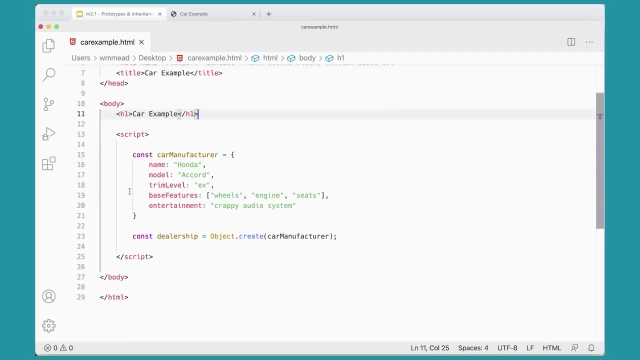 the name of the manufacturer, the model, a trim level and some base features and perhaps some other features like an entertainment system. So we've we've created that here And go over in your code editor and add this Type this out: 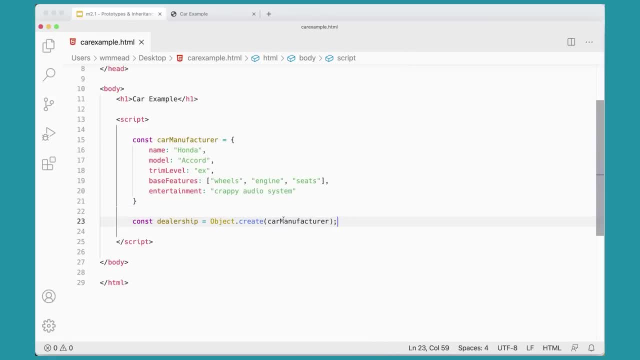 Add this script in here with this object. It's a good idea to type it so you get used to typing JavaScript and working with this stuff. So type this object. You can pause the video until you have car manufacturer typed in to a basic HTML file. 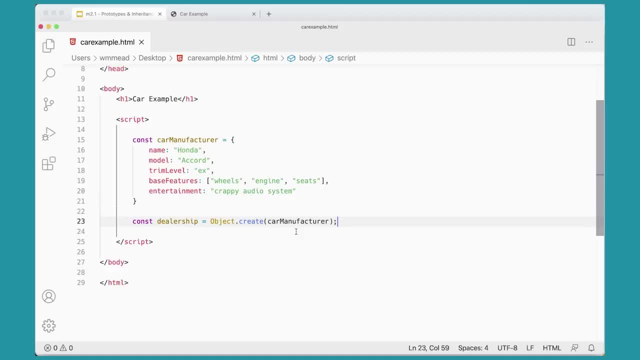 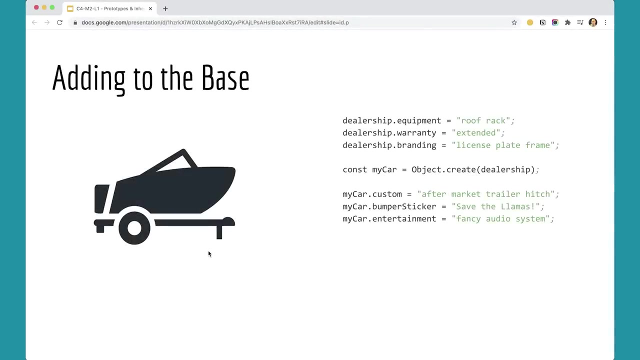 With the name, the model, the trim level, the base features and the entertainment system. Okay, great, Once you've got that, we can set up this variable dealership with objectcreate car manufacturer. The dealership gets the car from the manufacturer but then adds some of their own features. 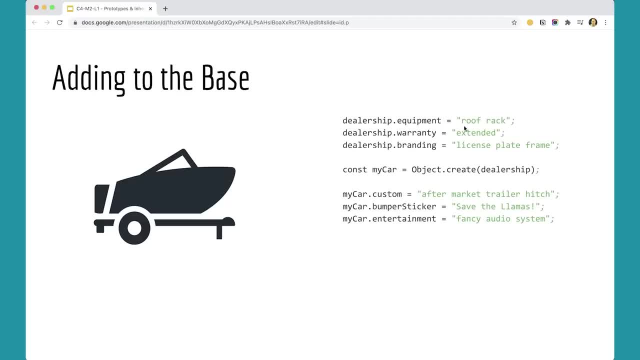 So, for example, perhaps the dealership adds a roof rack, or they add a warranty and it's an extended warranty, Or perhaps they put their license plate frame with their own branding on it around the license plate, So they've added that to the car. 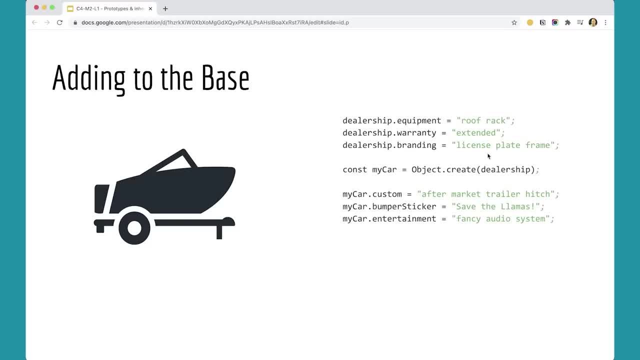 And let's go back to our code editor and add these items for the, for the dealer here, And then we'll add our own custom items to our car, which we'll get assigned a variable- my car, which is going to inherit from the dealership. 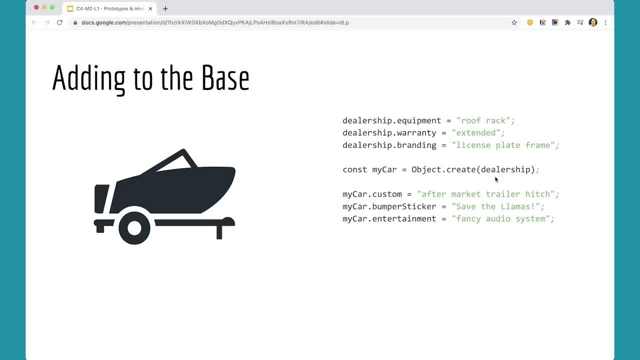 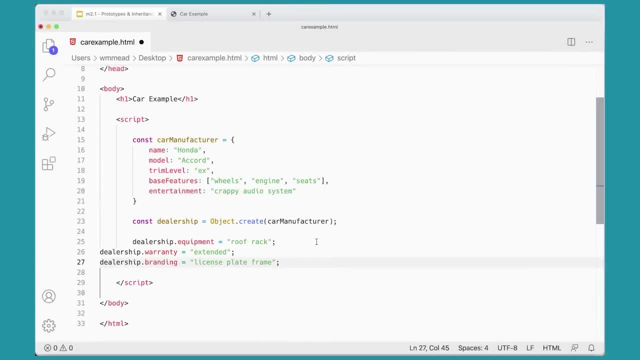 So now we've got sort of three levels of inheritance going on, So let's go over to our code editor and add this. So the dealership has added these features: Roof, rack, extended warranty and a license plate frame, And then from there 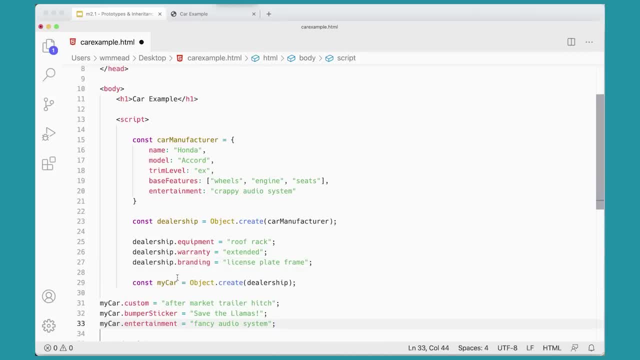 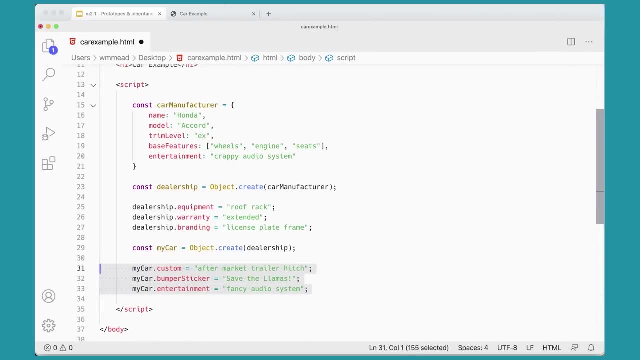 you get the car. So I'm going to make another variable: my car, which is going to create a object from the dealership object, And my car is going to have some custom things in it. It's going to have an aftermarket trailer hitch. 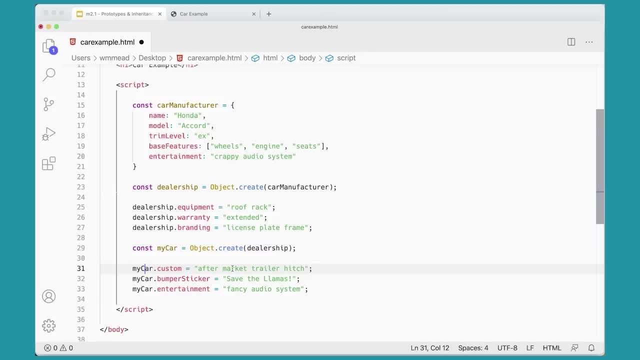 so I can tow my stuff. It's going to have a bumper sticker to save the llamas, because llamas are awesome, And it's going to have a fancier audio entertainment system. So notice, I'm upgrading the entertainment system that came from the manufacturer. 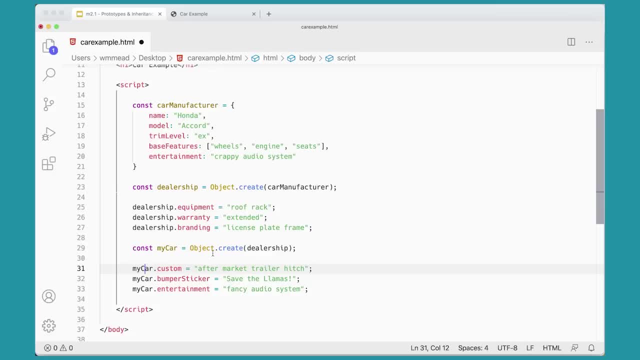 So that's great. So now we have a car that has sort of traveled through three processes. It was originally manufactured and then dealer got it and they added some stuff to it, And then I got it and added even more stuff to it. I can now access features of my car. 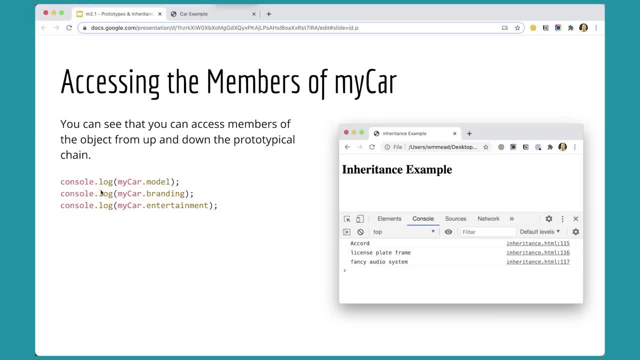 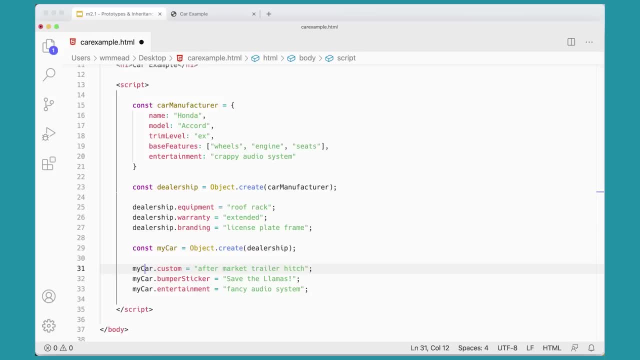 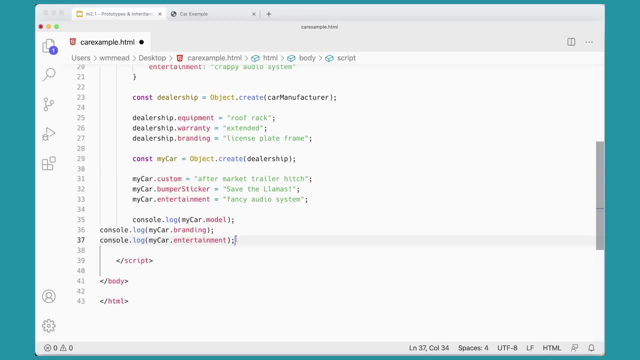 by using the console log and access different features up and down that entire prototypal chain. So let's go ahead and put this in over here And you're going to have to type it, but I'm just going to paste it in so you don't have to watch me type it. 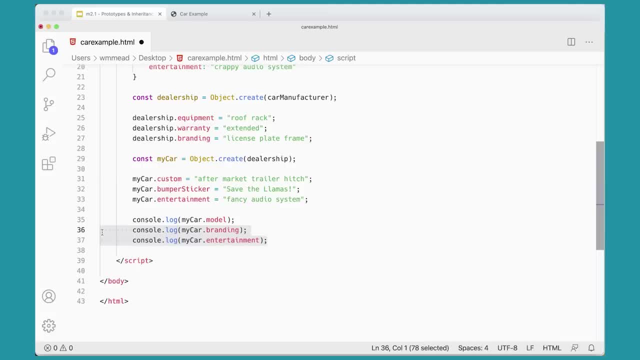 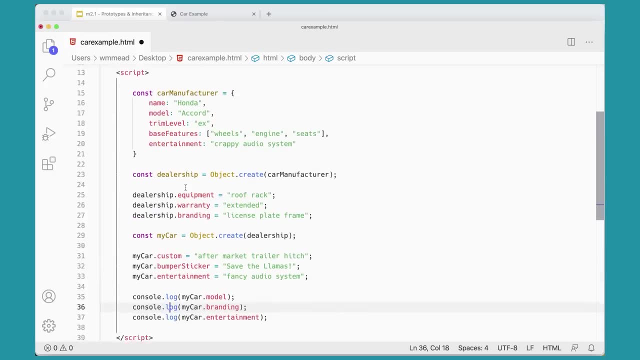 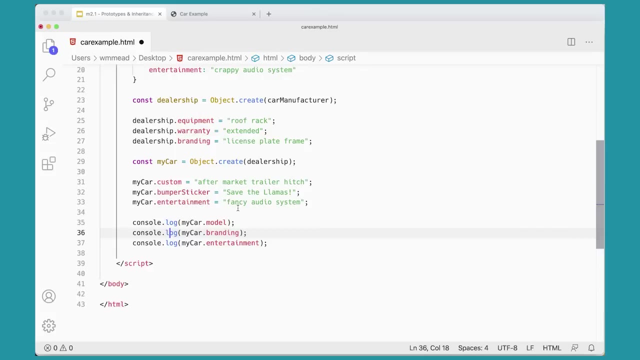 and make all the mistakes that I make when I'm typing Console log. My car model is going to go up to what came from the manufacturer, but branding comes from the dealer. and entertainment: it should give me the updated entertainment system. Let's see that it does. 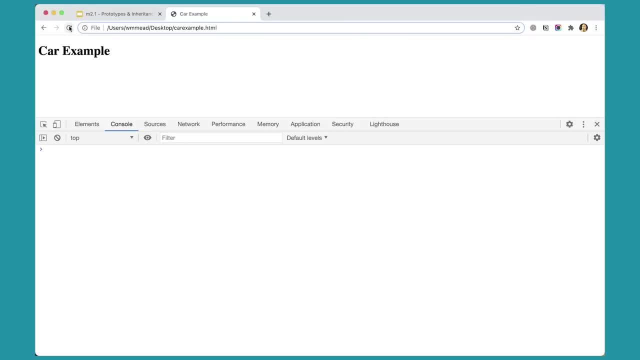 I'm going to save that and come over here and refresh this page And you can see that it's getting a cord, it's getting the license plate frame and it's getting the fancy audio system that I put in. So these properties work up and down. 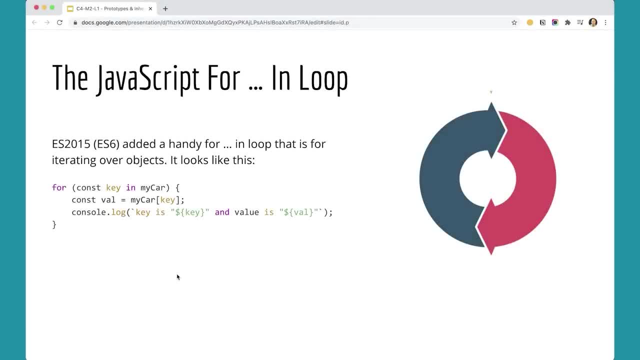 the prototypal chain ES2015 or ES6, added a handy for in loop, that's for iterating over objects, And it looks like this: Notice the in keyword here- And we've seen with arrays we have a for of loop where it's for and of. 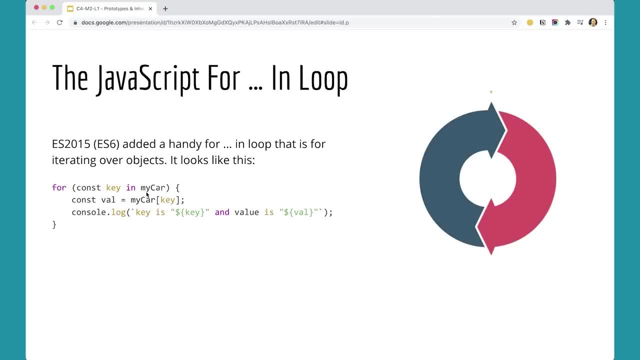 but the for in loop is specifically for objects, like my car, which is an object. So I've created a variable here called key And then down here I've created a variable called val, And it's going to be whatever key gets assigned here. 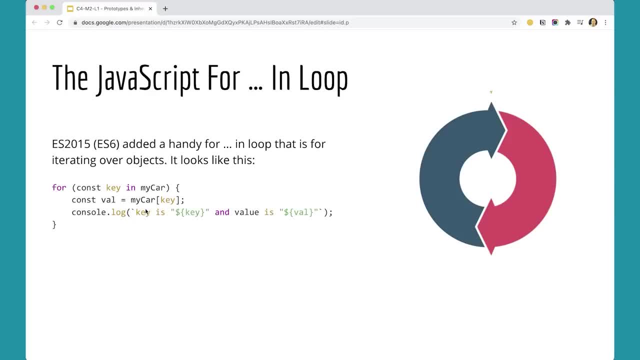 It's going to be. whatever value gets assigned here And I can see the key is the key and the value is the value, And what this should do- and we put this in our script- is that it should loop through this entire object and show all the things that I've added. 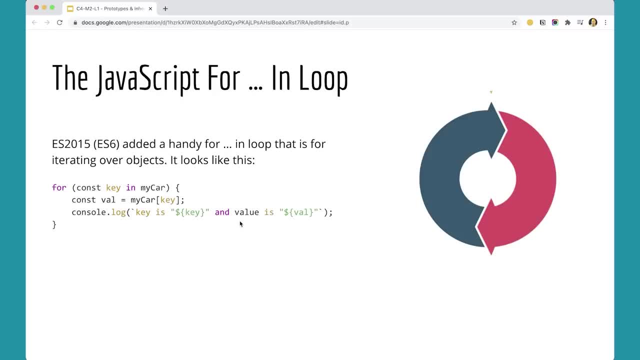 custom to my car, plus all the things that were inherited from the dealership, plus all the things that were inherited from the manufacturer. So the object should contain all of that. So let's go over to our code editor and have this to see how it works. 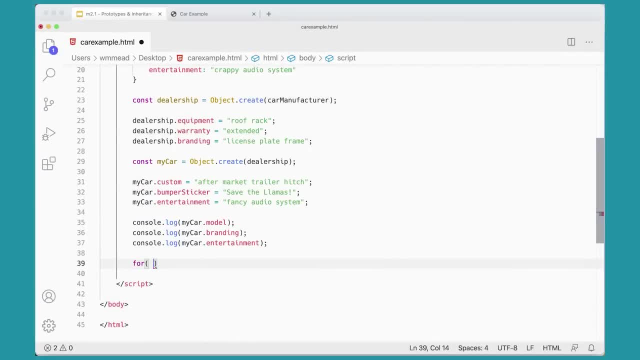 For const key in and then the name of my object- here my car, Like that- So I can go ahead and get, get the key, Get each key. I'm getting each key all the way up and down the prototype, Then inside the for in loop. 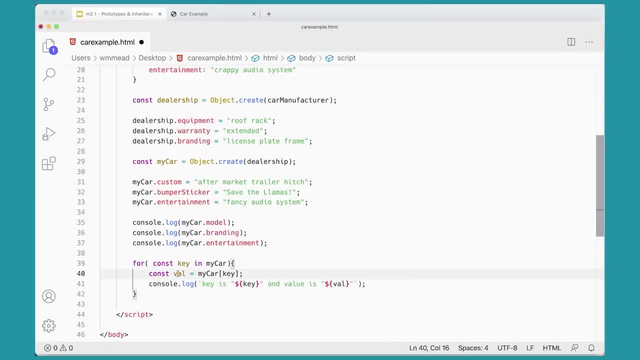 I'm just going to add a variable value that's going to say what is the key. So for each, it's going to go through this loop and get each key and put it in val And then I'm going to console log out. key is key. 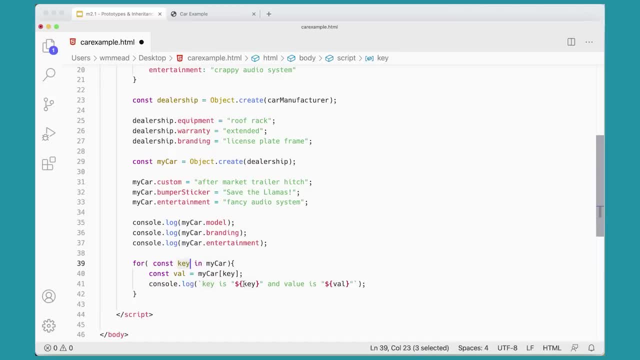 whatever the key is. That's this key here, And the value is val, And you can see that I'm putting that inside of tick marks using my object literal. So go ahead and do this and save it and then come over and test it out. 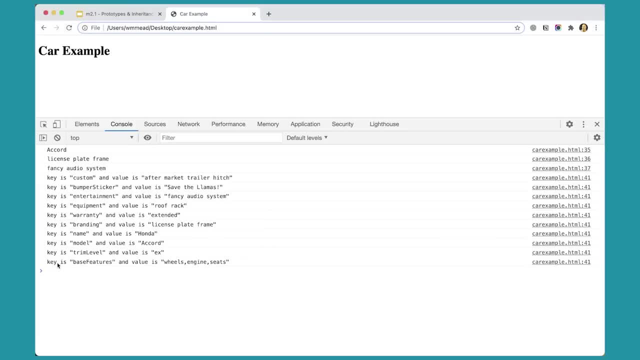 And you should be getting all of the keys custom And notice it's notice where it's starting. It's starting with. it's not going in reverse order. It's starting with the first item that's in the. that's directly on the object: on the my car object. 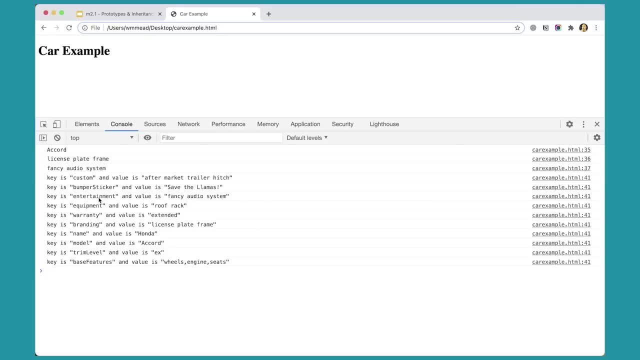 which is the aftermarket trailer. So this is the aftermarket trailer, So it's going through those first, Then it goes through the objects that it's inheriting from its prototype And then it's going through the objects that it's inheriting from its prototype. 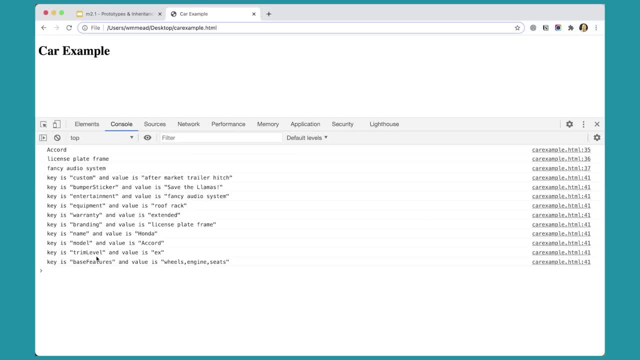 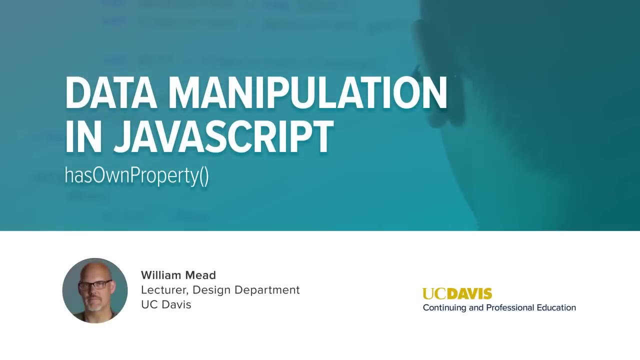 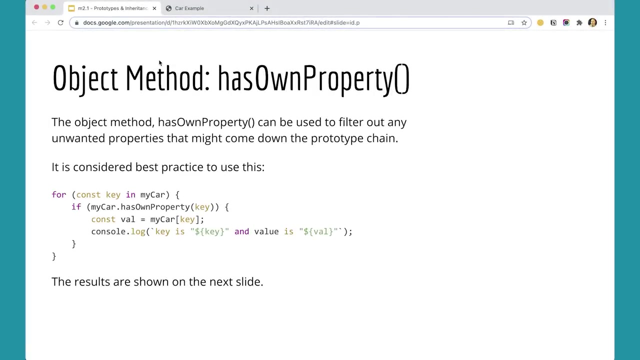 All in order here. So notice the order, because that's helps you understand the way that JavaScript is accessing the different properties. Frequently in real world programming situations, you don't want to inherit, You don't want to access the properties that are inherited. 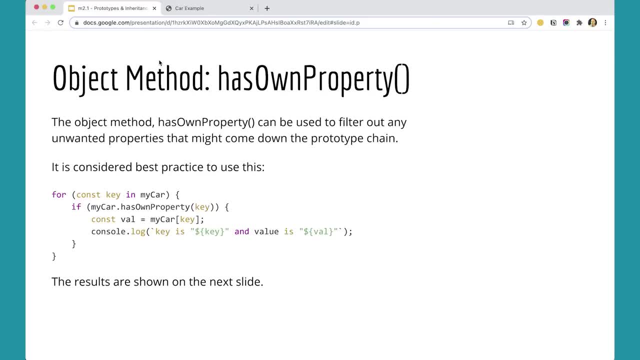 You want to access that particular object's properties and make sure that you're not getting properties from a parent- And this is frequently. a best practice is to make sure that you're working with the properties that are directly on the object and not ones that come down. 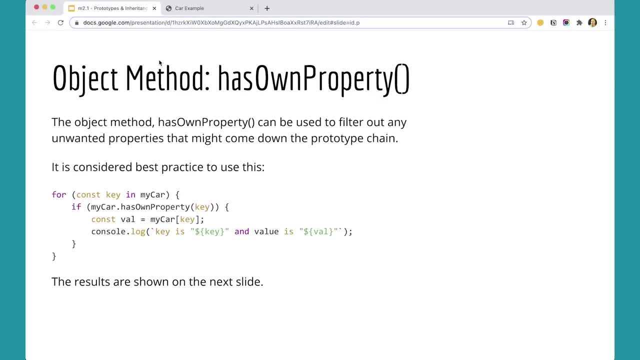 through the prototypical chain, And so we have a tool for doing that. It's called has own property, And we can check to see if the car has its own property and do that. So- and I'm mentioning this now because we're actually going to see this- 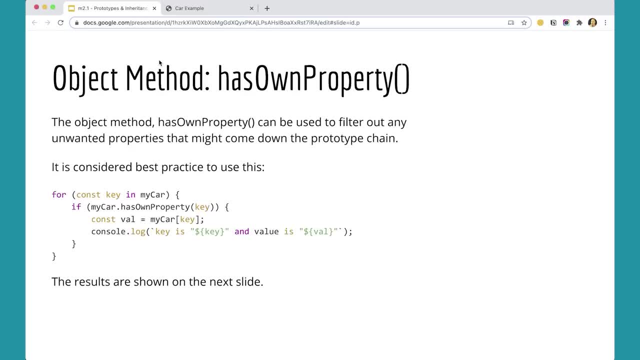 in a project coming up in this module. So that's why I'm putting this in here, so that you can see that we're doing this and to understand it in context of the theory of how it works. So, in order to get just the properties, 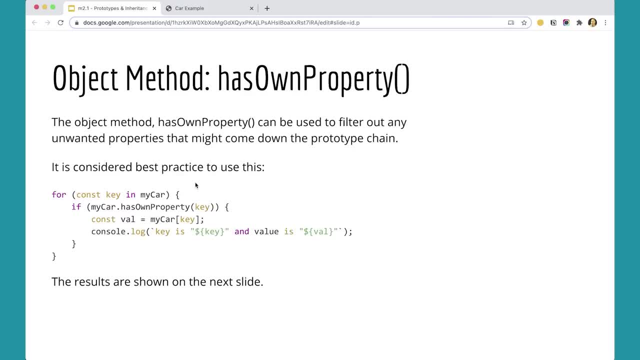 that are on the car and not the ones that are inherited from the dealer or from the manufacturer. we can use the has own property method here to do that, So let's go ahead and do that over here. So in here I'm just going to add an if statement. 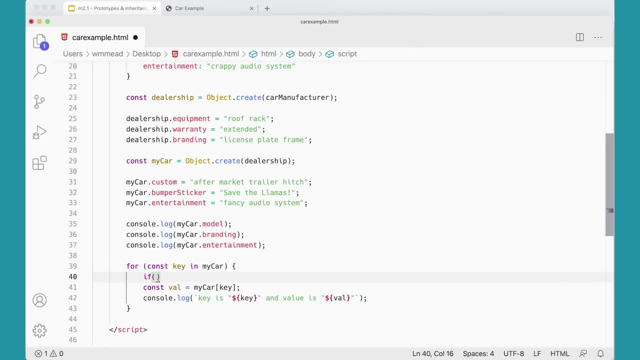 If my car dot has own property and I'm going to put in key, So if the key belongs to the car, if that's true, then I'm going to do this stuff, I'm going to put in there. Maybe I'll comment this stuff out. 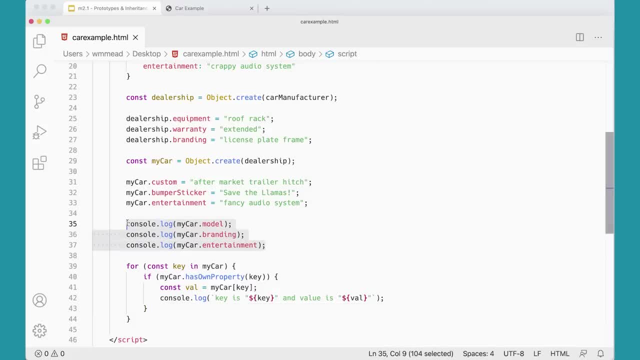 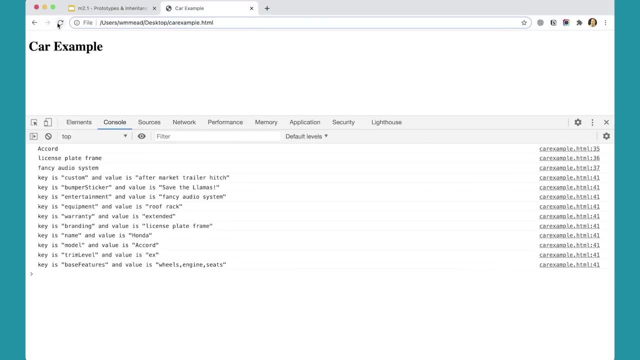 so I don't get that polluting my console log. There we go, All right. So now, if I go and run this file, you'll see, instead of getting everything here, I just get the things that belong to my car: The aftermarket trailer hitch. 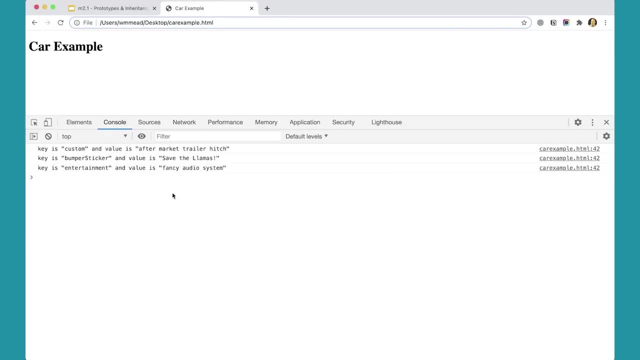 the Save the Llamas bumper sticker and the fancy audio system. And again, frequently in real world projects, you want to make sure that you're only working with the properties on the object itself and that you're not working with properties that have been inherited. 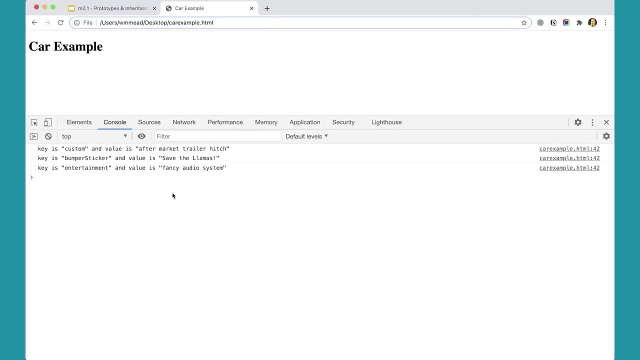 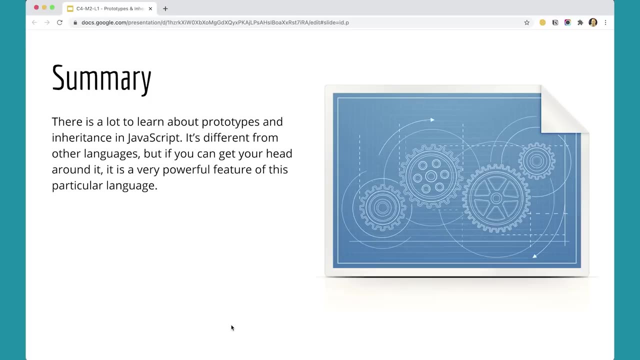 through the prototypical inheritance chain. Summary: There's a lot to learn about prototypes and inheritance in JavaScript. It's different from other languages, But if you can get your head around the ideas, it's a very powerful feature of this particular language. 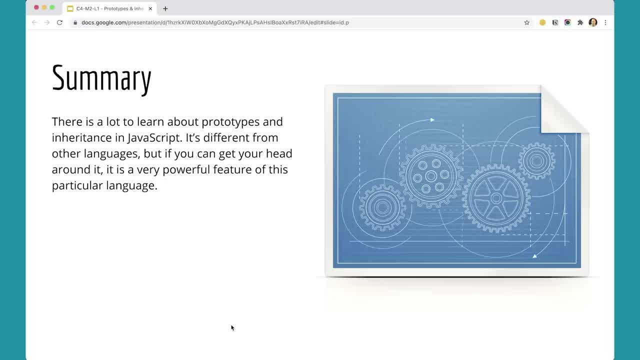 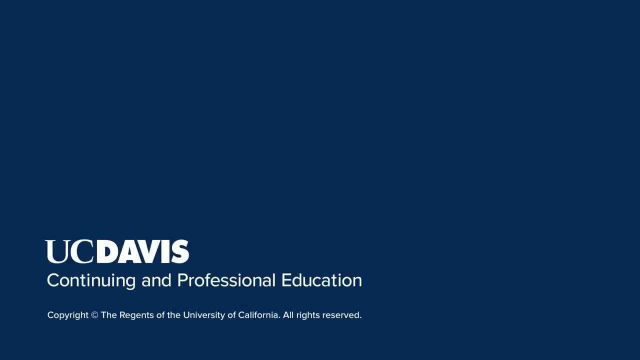 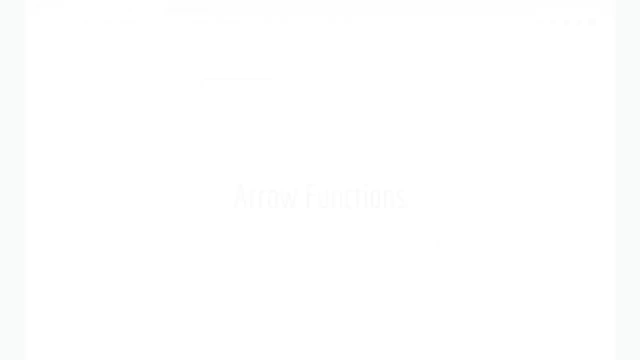 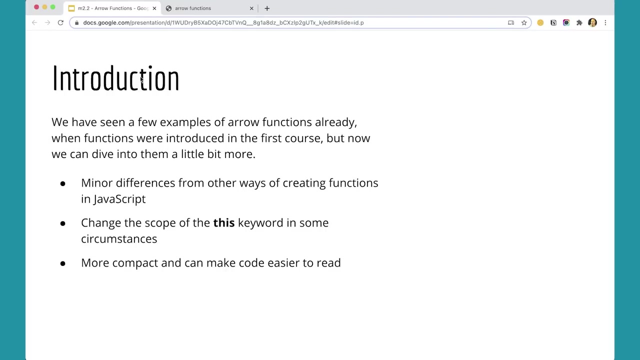 The way prototypes and inheritance and the way functions work in JavaScript is a really great combination And we're going to see that in some projects coming up Arrow functions. We've seen a few examples of arrow functions Already, back when we first introduced functions. 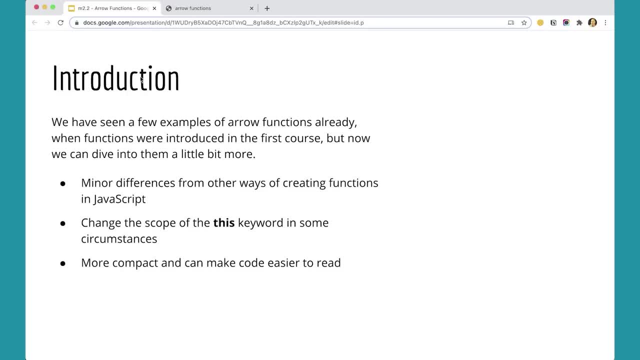 in the very first course in the specialization. But now it's time to dive into them a little bit more And for the most part, arrow functions are just a slightly different syntax for writing functions. There are some minor differences from other ways of creating. 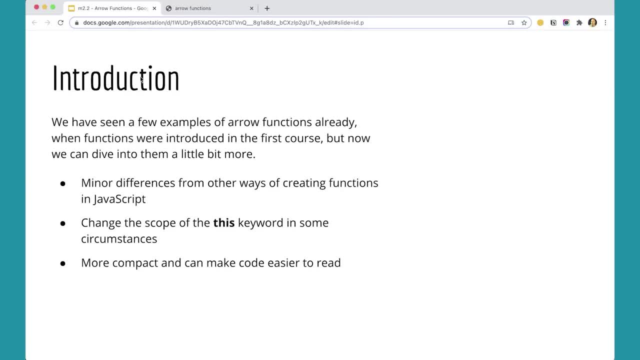 functions in JavaScript, particularly things like the scope of the. this keyword in some circumstances is different And we'll see an example of that, But they're more compact and they're and they make code a little bit easier to read when you use them appropriately. 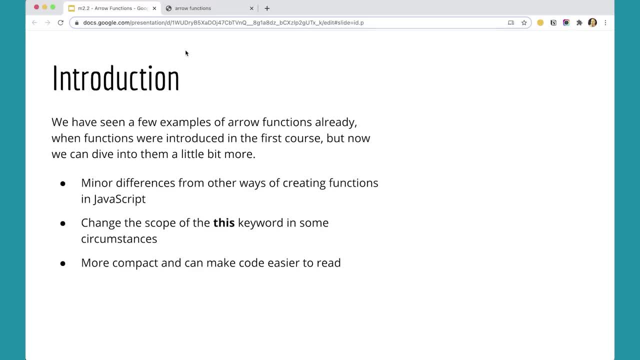 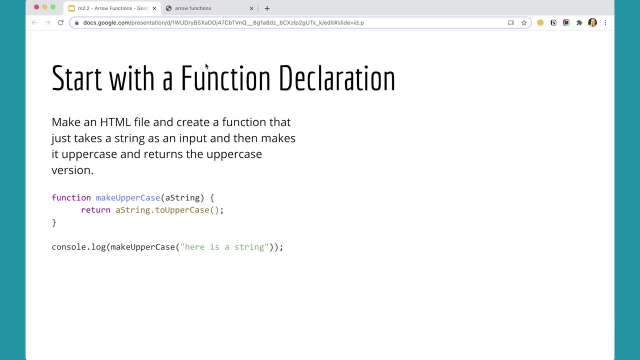 So let's take a look at some examples of how to do this. To start with, just create a file, an HTML file, and add a function that takes a string as an input and makes it uppercase and returns the uppercase version. So let's go over to our code editor. 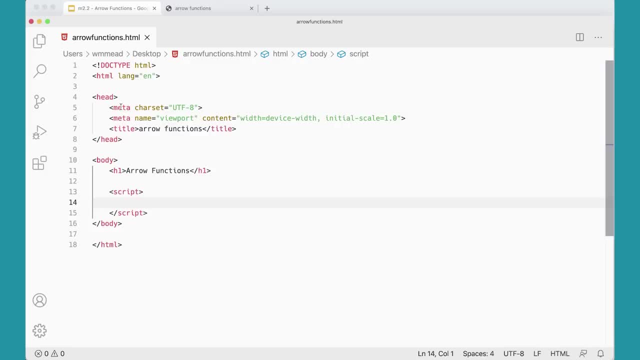 and add a function that does this. So here I have just a basic HTML file with arrow functions and an h1 and a script tag here. So go ahead and make this HTML file And then I'm just going, I'm going to just paste this in. 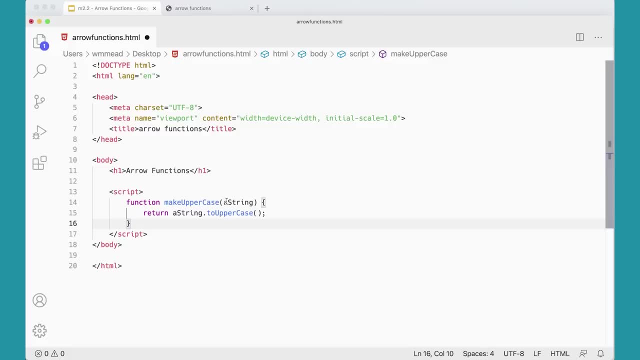 But you can type it function make uppercase a string. It takes a string as input and then we return that string as output. So down here I could do consolelog, make uppercase And then in there I'm going to pass. in here is: here is a string. 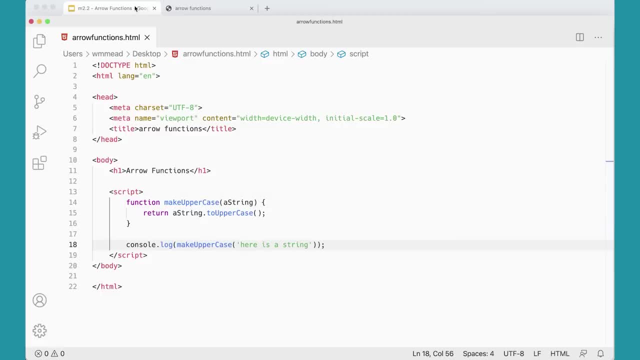 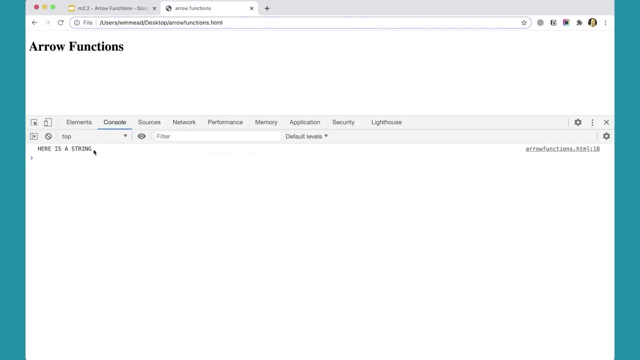 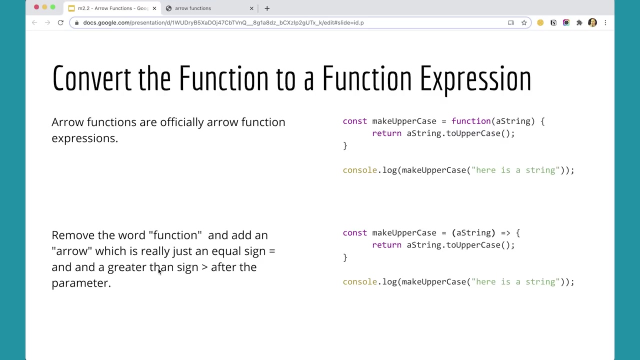 All right. So now, when we run this over here, we get here is a string all uppercased. So that works, That function works And that's a function declaration. That's the kind of thing that we're used to doing. Now, first thing to understand. 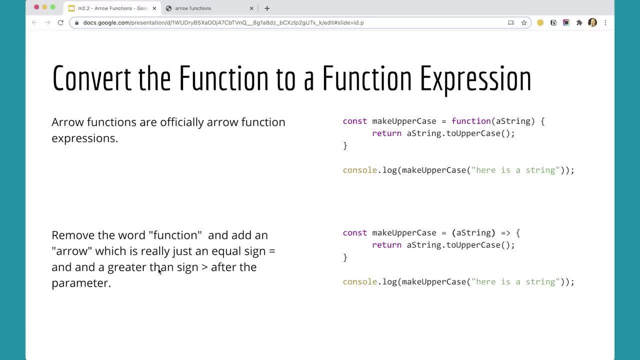 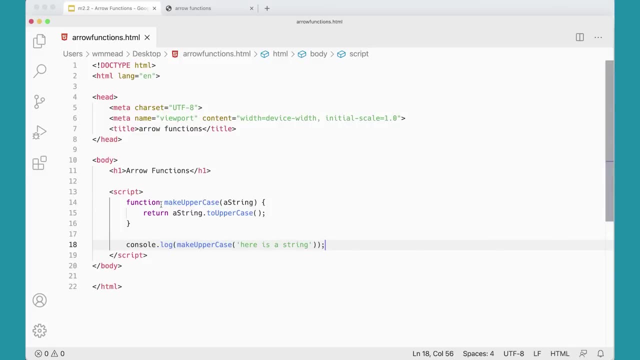 is that arrow functions are function expressions, So the first thing to do is to convert this function from a function declaration to a function expression. So let's do that really quickly And it'll really help you to get used to this syntax to actually do this stuff. 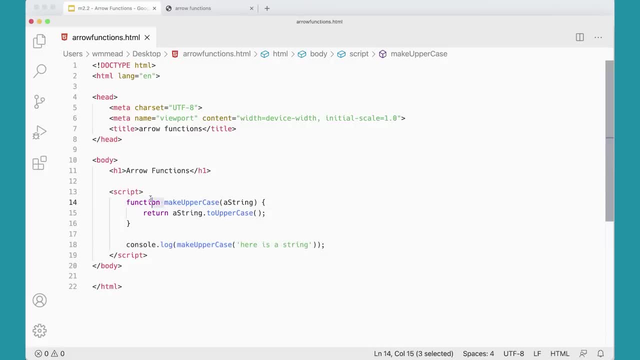 So instead of putting the function keyword here, I'm going to say const- make uppercase equals function, which takes a string and returns that string. So, like that, make uppercase, And then, and that's it, And so this is a variable, So this is a function expression. 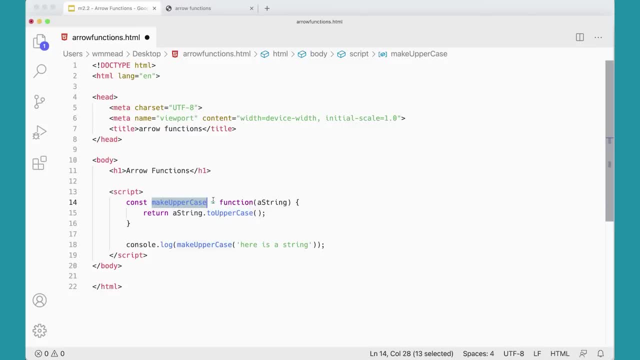 because we're using the equal sign. So it's an expression. We're assigning to this variable this function that returns the string there And that should work exactly the same way. If we come over here and run this again, we get- here's a string: uppercase. 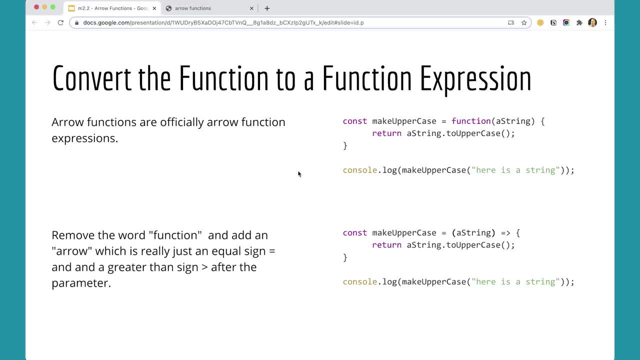 So then, the next thing we want to do is convert it to an arrow function, And the way we do that is we remove the word function and replace it with the equal sign and a little greater than sign here on this side of the expression. So let's do that. 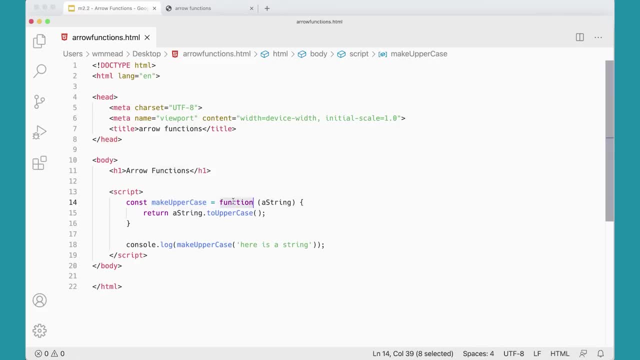 So down here, instead of function here, we take that out And instead we put in over here an equal sign and an arrow like: so Equal sign and the greater than sign, And so this is an arrow function. We remove the word function. 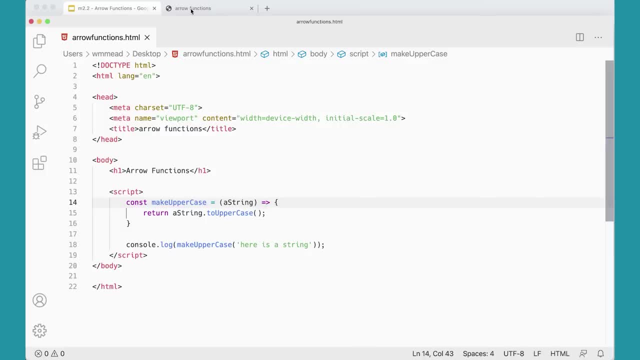 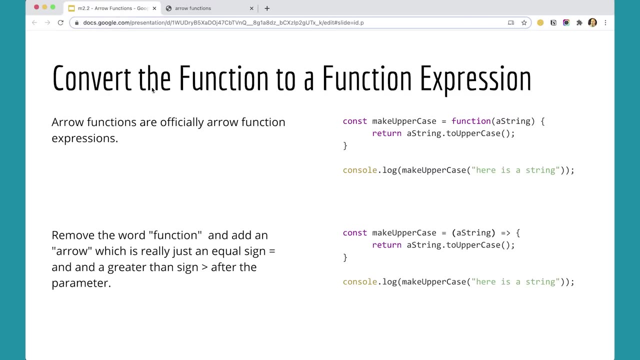 and we stuck in the arrow over here, So that should work just the same way. Let's go back and check. If I refresh I get. here is a string all uppercase, So that's working exactly the same way. Now, beyond that, 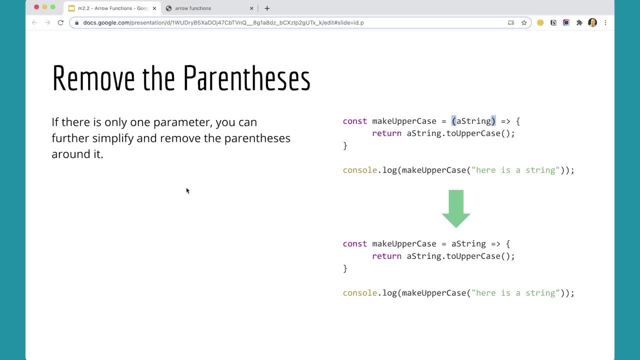 we can. if there's only one input going in, we can actually get rid of the parentheses around that one variable, Just as another way of saving space. If there's more than one variable, then we would have to leave them there, But if there's only one variable, 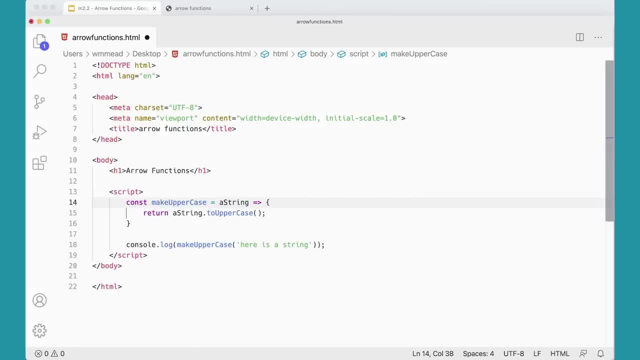 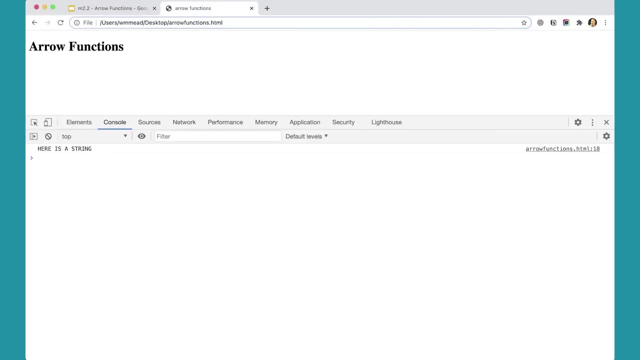 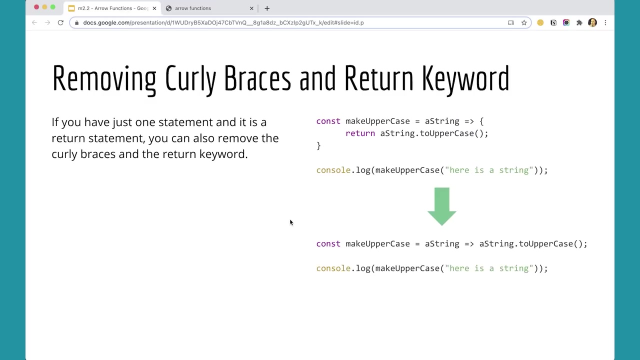 we can actually get rid of these parentheses, So you can make it even shorter. If we come back and run that again we get here is a string. So that works, That's great. So we've got that in there. Now even further. 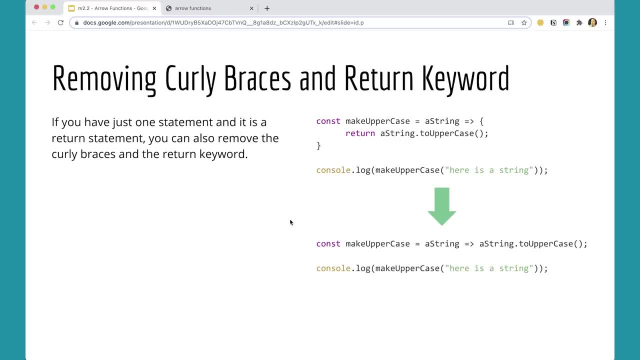 because this particular function does only one thing: it returns a value. we can actually remove the return keyword and the curly braces as well, So we can actually shorten this whole expression down to one line with the arrow function in this particular case. Because this particular function. 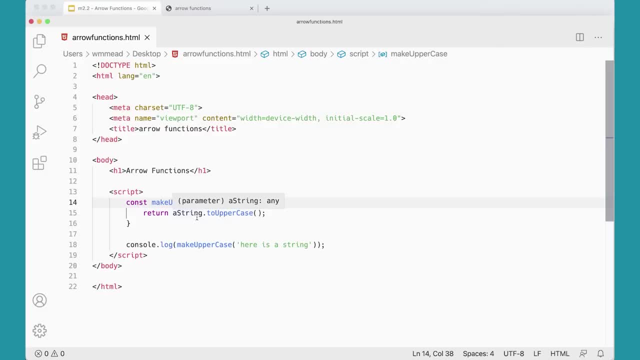 does only one thing and it does a return thing. we can do this Now. if it did other things, additional things, we'd need to leave the curly braces. Or if it did more than just return something, we'd need to leave the curly braces. 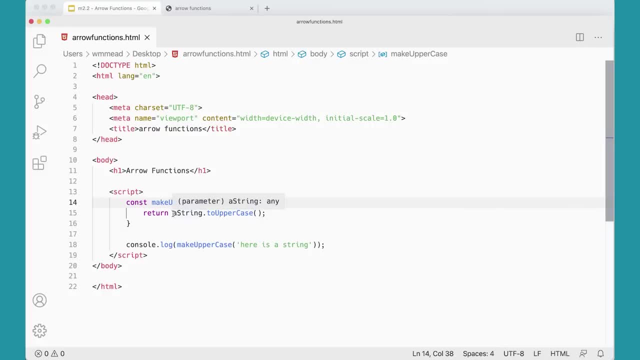 But because it doesn't in this case we can actually just make this, say that. So it's down to one line And, if you look at it, we're making a variable, make uppercase, and it's assigned, it's taking an input. 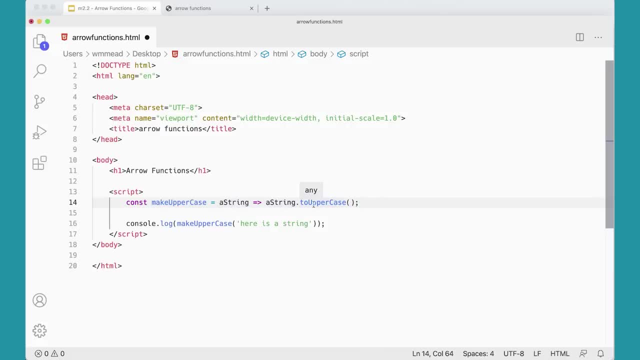 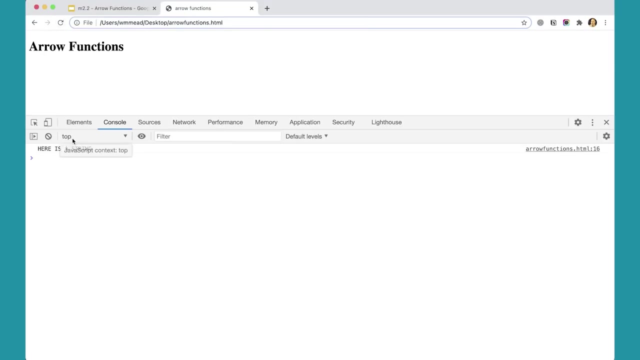 and taking that input and making it uppercase. So if you can get used to the syntax, it's actually very readable once you get used to it. So let's save that and then come back and run it again And we get here as a string. 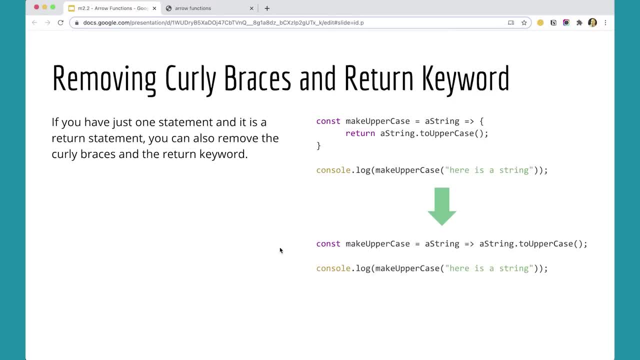 So that's a pretty interesting way of making use of arrow functions. Again, if you needed to do more than just one thing, you'd need to leave the curly braces in there. If you had more than one input, you'd need to leave. 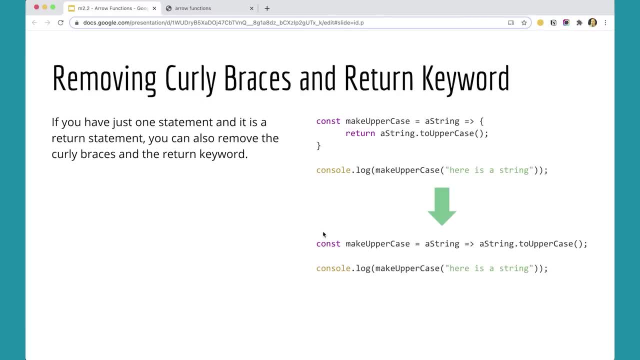 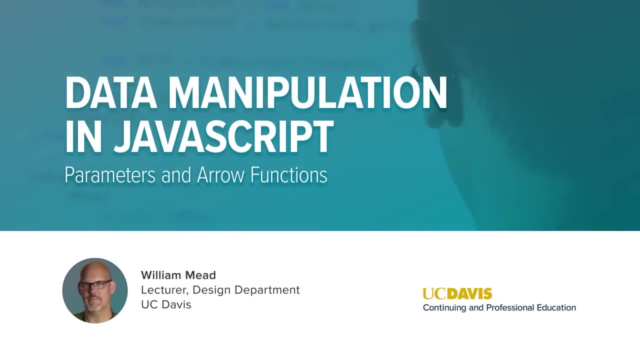 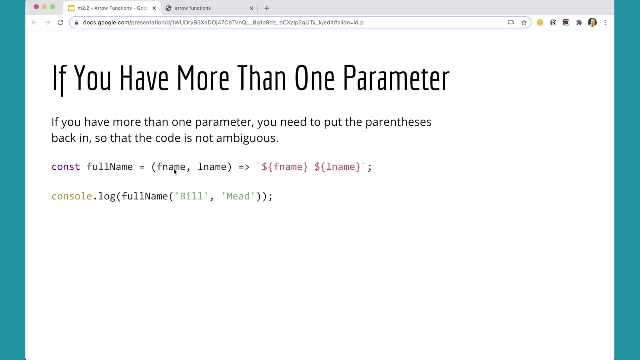 the parentheses in there, But there are possibilities for shortening down this function expression into just one line, which is pretty amazing. Here's an example with more than one parameter, So I'm passing in first name and last name and then I'm just returning. 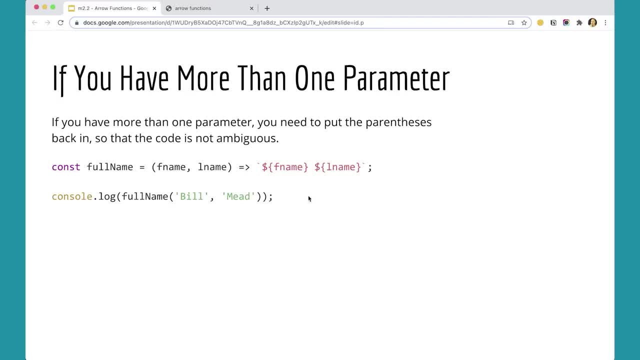 the first name and last name together in a string, So we could actually consolelog like that, And that's maybe a situation where you might use this type of thing, So let's go ahead and put this in here, just to see what that looks like. 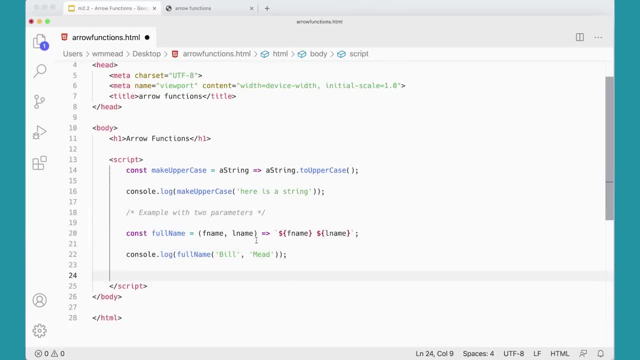 And you should type it. Make sure you go in and add this and type it in here: const: fullname equals the full name in there And then go ahead and put that in there. So I'm going to save that And then you'll see over here. 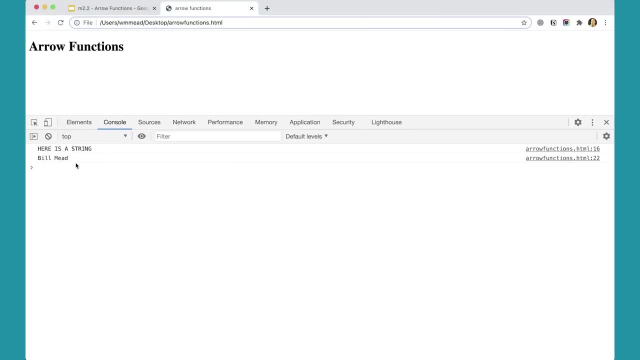 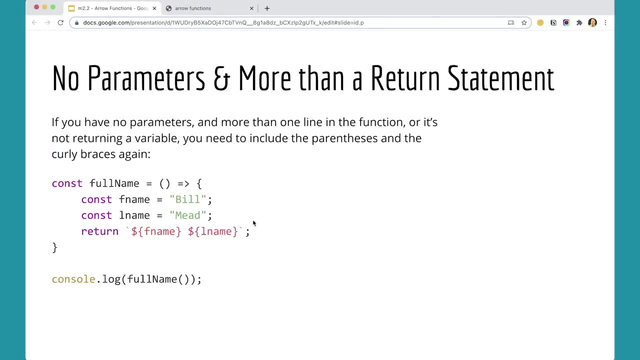 if I refresh this, that I get my full name coming back returning here, So that's great. We could also talk about no parameters and more than a return statement. So this version of full name doesn't take any parameters, It just gives you the full name. 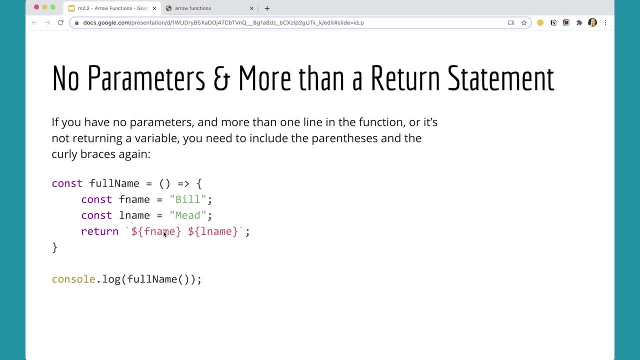 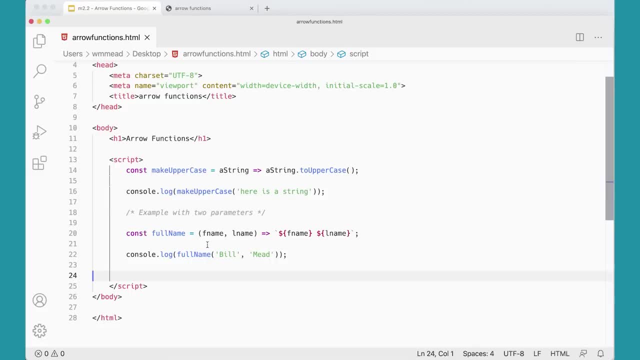 that's built into the function, which is perhaps less useful than the previous example but worth taking a look at really quickly here. So let's go over to the code editor and change this to const fullname equals, And then we're going to have 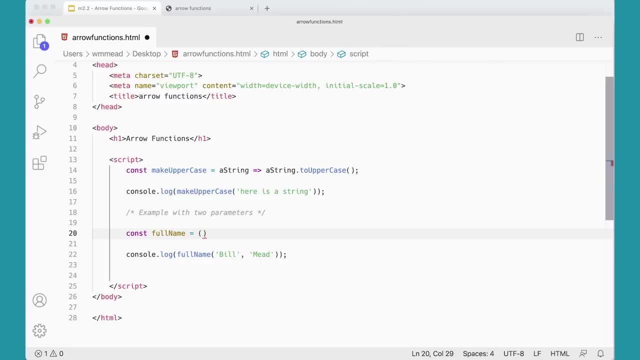 just parentheses, because if you're going to not have any parameters at all, you have to have the parentheses for clarity here, for what this thing is doing. And then we're going to have our error function here: equals angle bracket. And then, if we're going to do 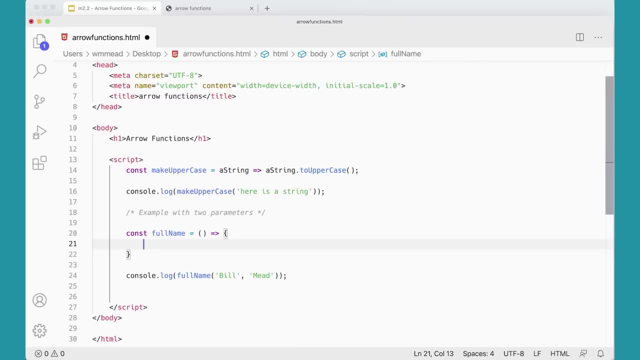 more than one thing, then we need to do something with the curly braces there. So now I could do const first, our fname equals bill, like so, and const lname equals quote mead, like so, And then I could actually do the return statement that I had before. 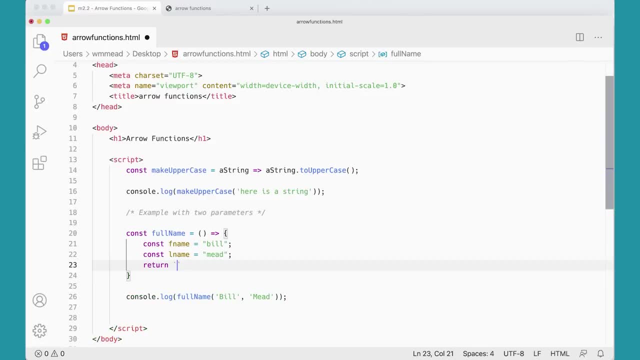 with the tick marks and the dollar sign curly brace- fname: curly brace. space dollar sign: curly brace- lname: curly brace, like so. So now console log: full name doesn't get any print, doesn't get any parameters at all. But you'll see that'll work. 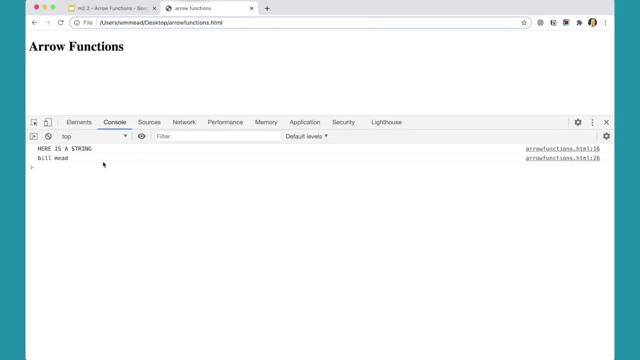 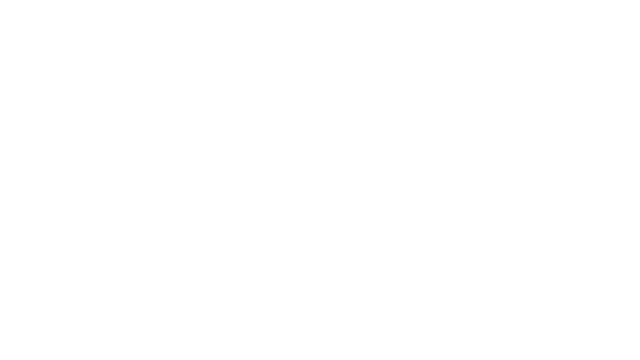 I made it lowercase so you can see the difference, But it is still doing the same thing. It's just in the second case we're doing more than just a return statement in here. That's kind of important to pay attention to When to use arrow functions. 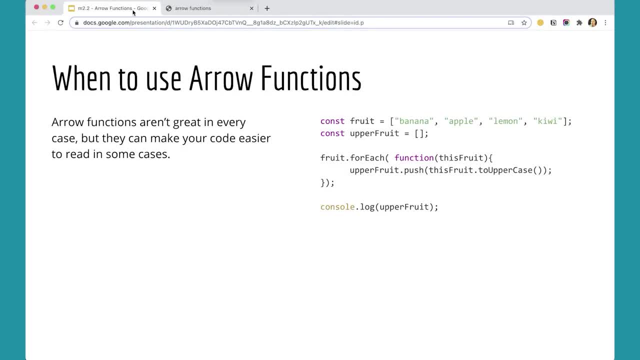 Arrow functions aren't great in every case, but they can make your code easier to read in some cases, And look for places where you have return functions or you have functions that are parameters, And those are often places that can work well for arrow functions. 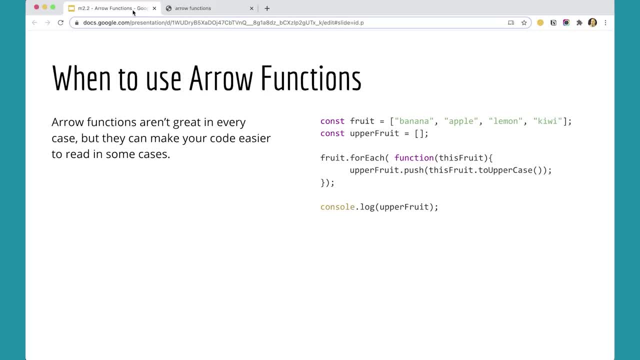 and to make your code a little bit more readable here. So, for example, over here I have a variable that is an array that has these elements in here, And then I have an array that's empty, And then I'm going to loop through each of the elements. 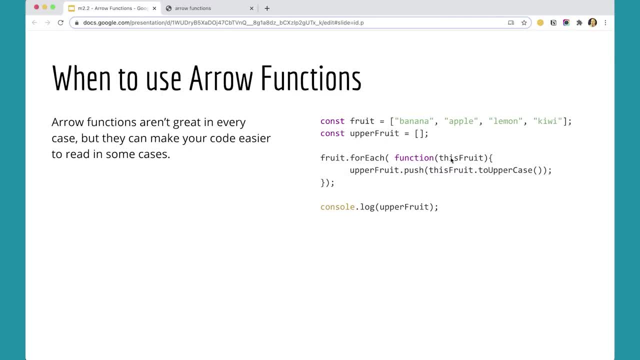 in the fruit. I'm going to do a foreach on those and run a function for this fruit that puts that, makes that fruit uppercase and then pushes it into this array And then I'm console logging out the upper, uppercase version. So we end up with two arrays. 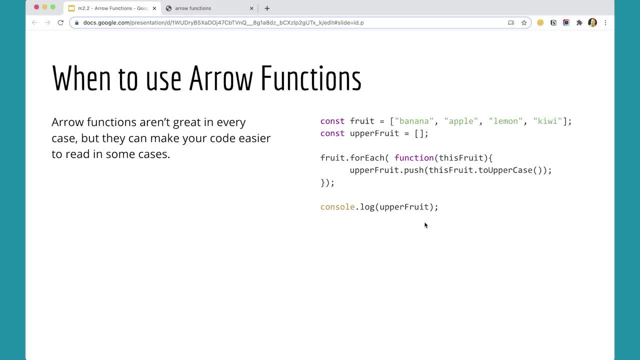 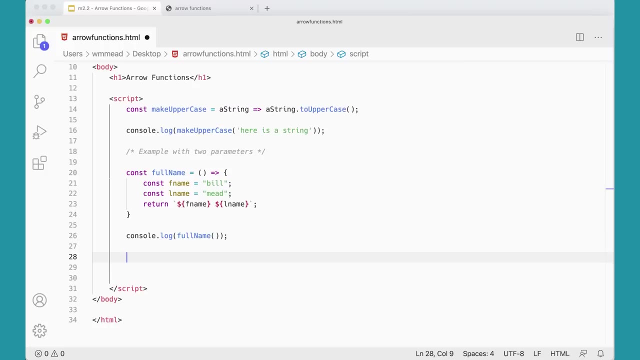 one with lowercase fruit and one with uppercase fruit. Not super useful, but a good demonstration of this. And can you take this function and turn it into an arrow function? So let's go over to our code editor. Make sure you type in this code: 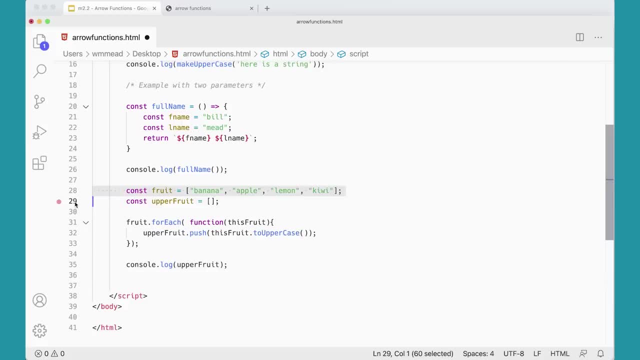 Add the array with the fruit, An empty array for upper fruit, And then add the foreach statement pushing that in. Okay, And again, the way to do this- I'm going to take this off for a second Foreach- is a method like so: 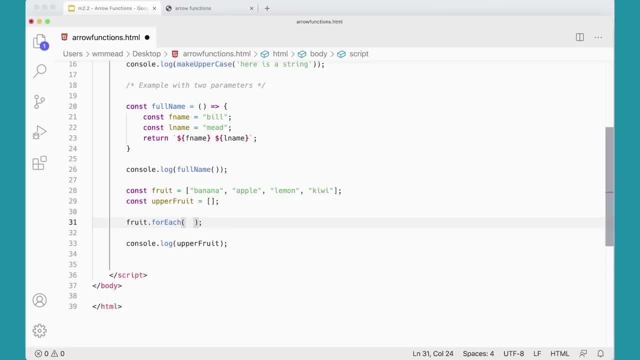 And it takes a function like so, And in this function we're going to pass in each fruit. And then what are we going to do with each fruit? We're going to say each fruit. Actually, we're going to say upper fruit. 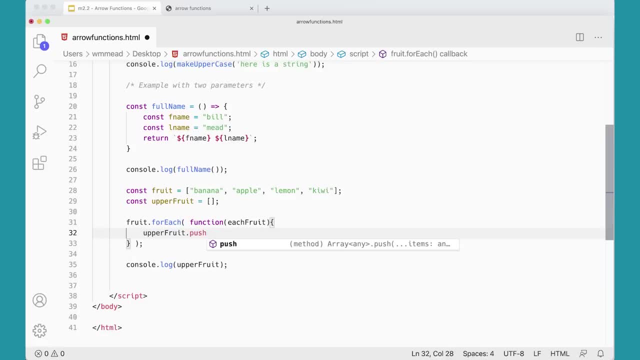 Upper fruit dot push. And then we want to take each fruit and make it uppercase. Each fruit To uppercase, So type it like that, Type it from the outside in. But how could we make this function? Let's just check to make sure this works. 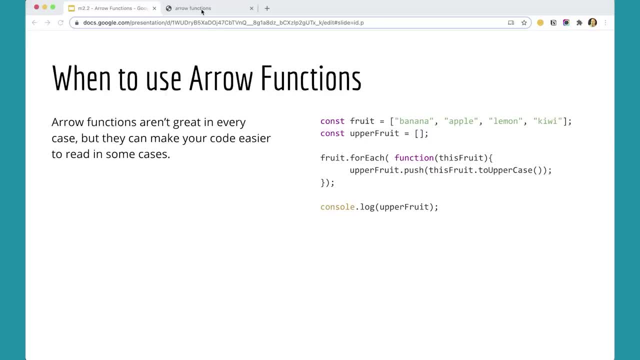 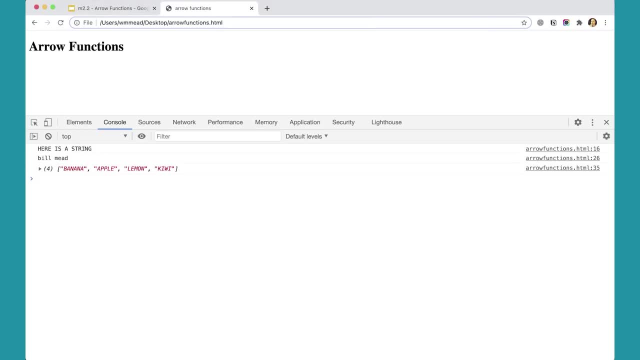 because this is going to console log out the upper fruit. Make sure I did that right first, And there we get uppercase fruits. So that's great, Okay, cool. So now, how can you take this function here and make it an arrow function? 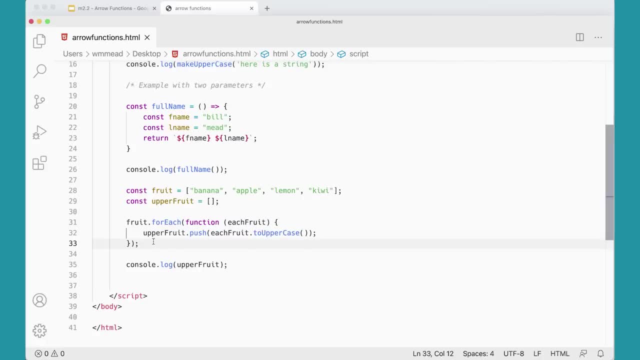 See if you can do that on your own. Pause the video and then see if you get the result that I get. This is how I would do it: Remove the word function and put the equal sign and the greater sign there. That turns it into an arrow function. 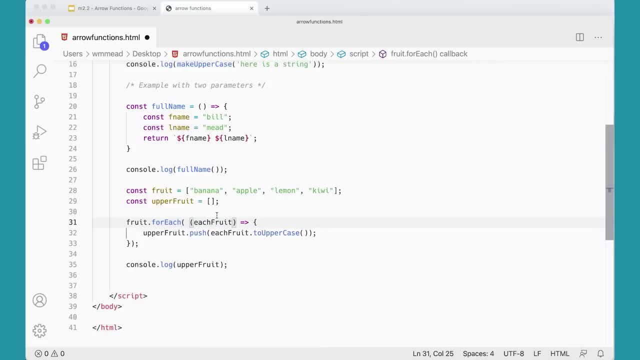 Now, because we have just one parameter here, this can be removed. These two parentheses can be removed Just for the sake of simplicity. Gets rid of two characters, So we can push that into upper fruit here And this is not a return statement, so we need to keep the curly braces. 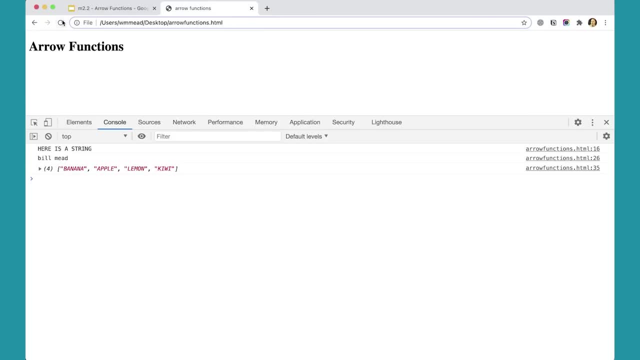 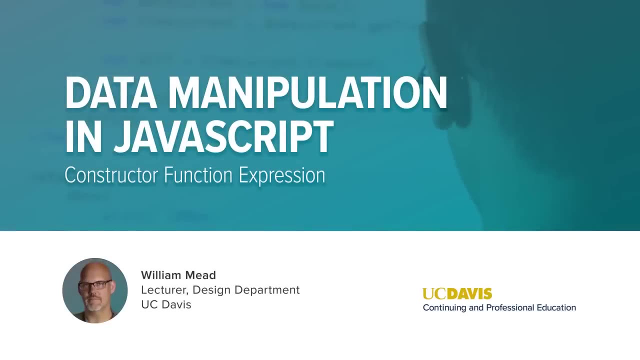 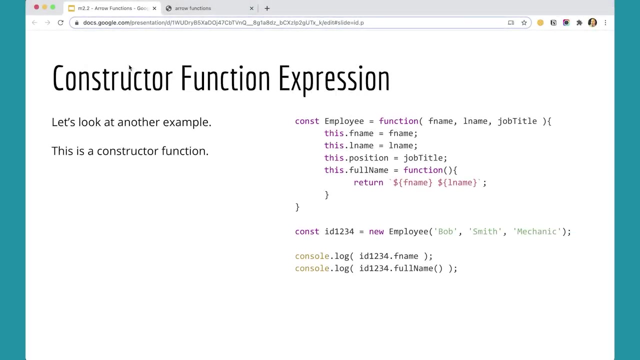 Check and make sure that works, That I did that right And sure enough, it works fine. Here we have a constructor function expression, And this has a good place where we can use our arrow functions, And so what you should do is type this out: 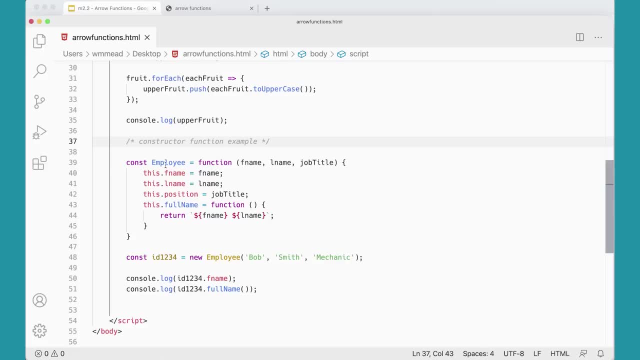 Add this to your example page. I have already put it on my page over here. So add this constructor function here. const employee. So we've got a variable called employee And it has a function that takes name, first name, last name and job title. 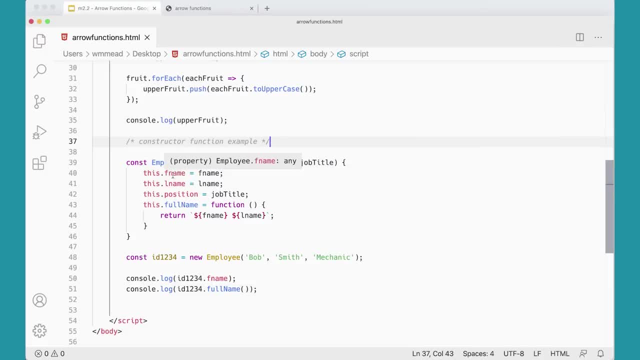 And then I'm using this keyword to set first name to whatever gets passed in here, To set last name to whatever gets passed in here. So you get a position to get whatever gets passed in here And then I've got full name. is running a function. 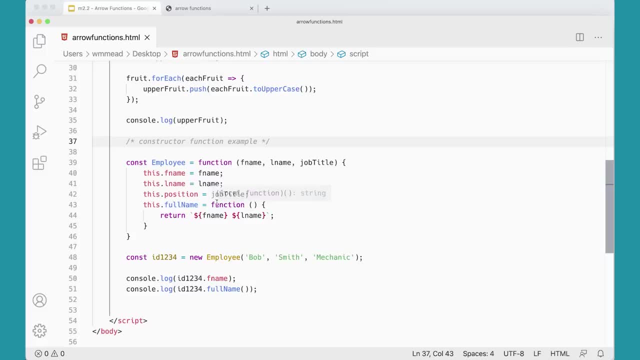 that's going to put together the first name and the last name. This function here is a good candidate for a function expression. So see if you can turn this function into an arrow function here. Go ahead and pause the video and see if you can do it. 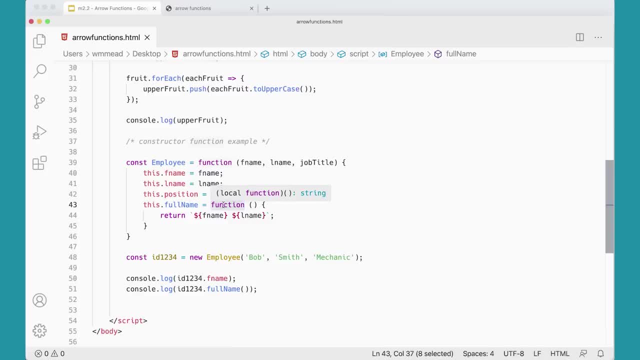 This is what I come up with: Remove the word function and stick an arrow here. equal sign angle bracket, like so We need to keep the parentheses because we're not passing anything in. But since it's only a return statement, we can actually remove the curly braces. 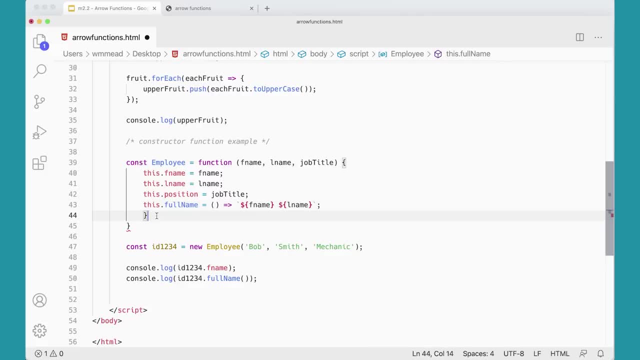 in the word return And you can see that this is now a shorter piece of code. that's kind of easier to read. This full name is a function that returns the first name plus the last name. It's kind of nice and easy to read that way with the arrow function. 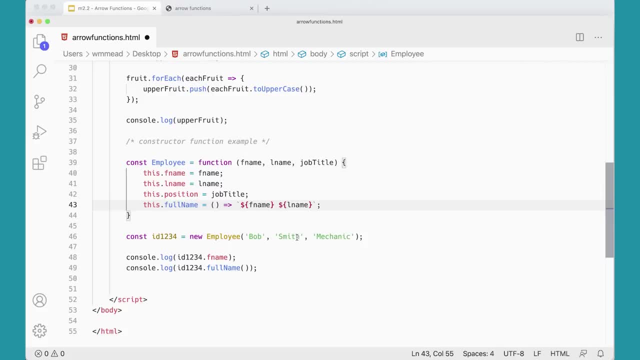 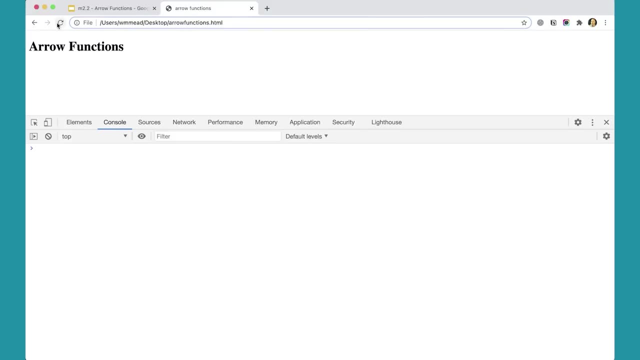 And it's shorter, So it's kind of nice if you can get used to using it. Okay, great, So we've done that and now we can come over and we can test it over here And you can see that I'm getting Bob. 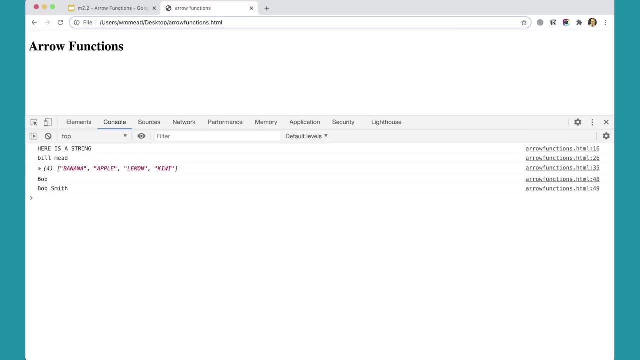 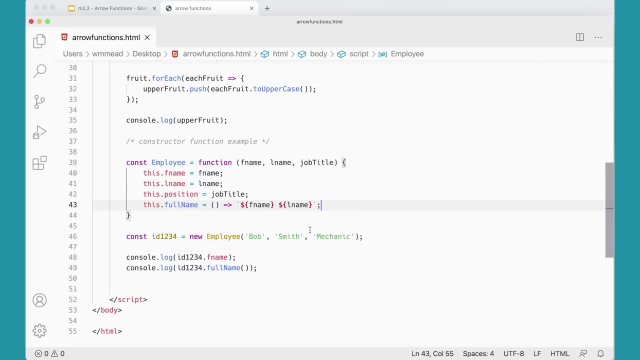 and I'm getting Bob Smith. I'm getting Bob because down here I have new employee, Bob Smith, mechanic, and I'm console logging out ID first name, fname, and then I'm console logging out ID full name. So I'm actually running that full name function. 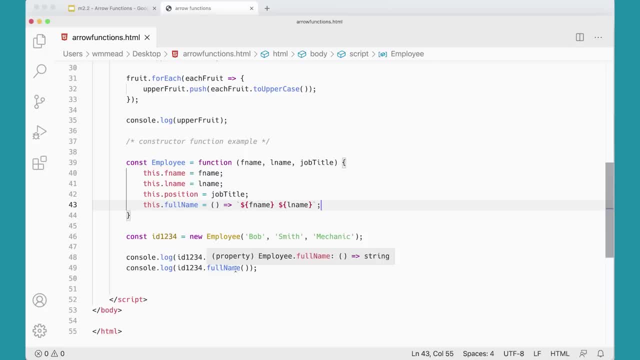 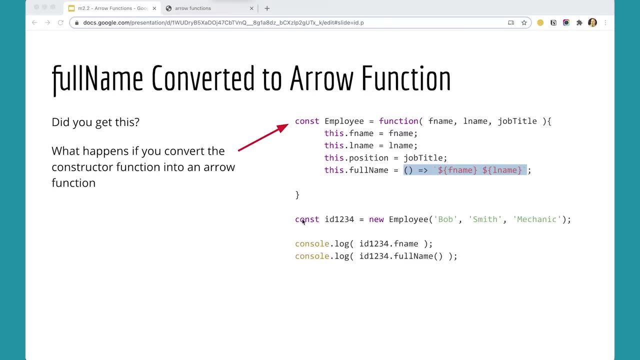 So I'm getting Bob for this and Bob Smith here for that one. Hopefully, you got something like this. And one thing that we can't do is convert this function into an arrow function, And it has to do with the way that this keyword is. 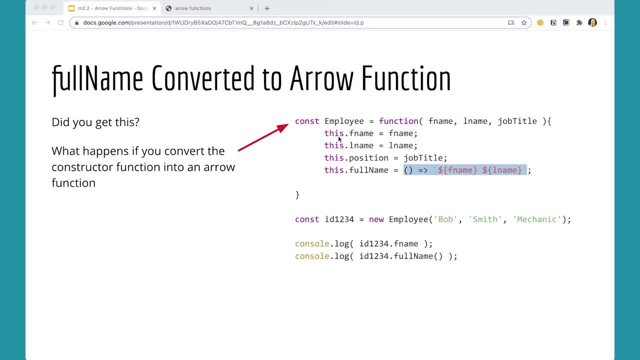 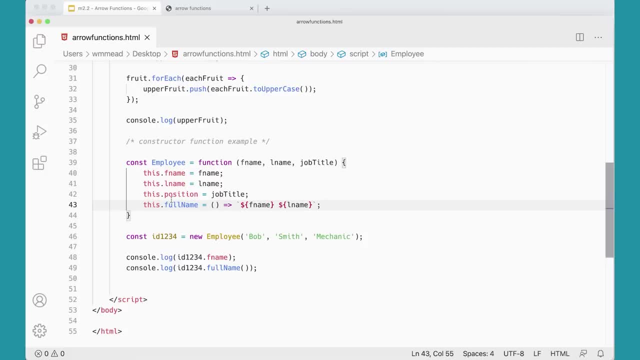 scoped. The scope of this keyword is different in arrow functions, And so let's give it a try, just to see the kind of error that we get if we try to do that. So over here, if I get rid of the word function, I have to keep the parentheses because I'm 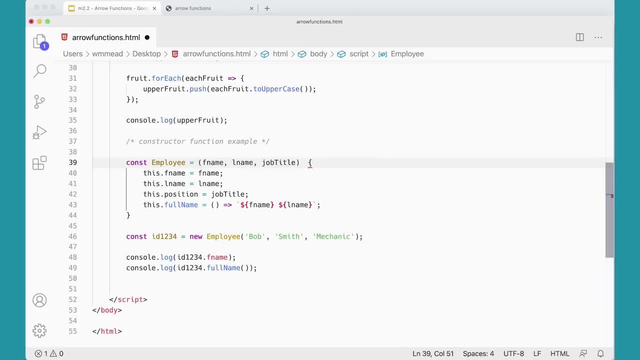 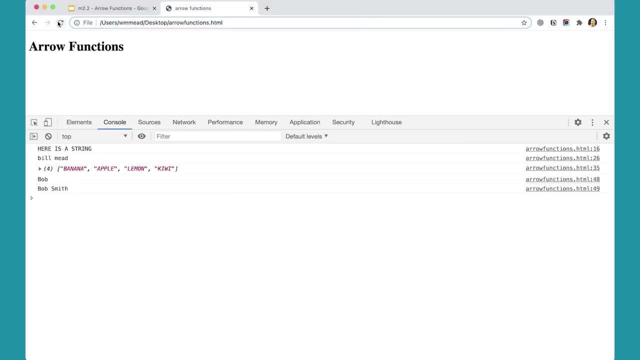 passing in three things and I have to keep the curly braces because I'm doing more than just a return statement. But if I put my arrow in there and then try to run this, you'll see that I get an error, Uncut error. Employee is not a constructor. 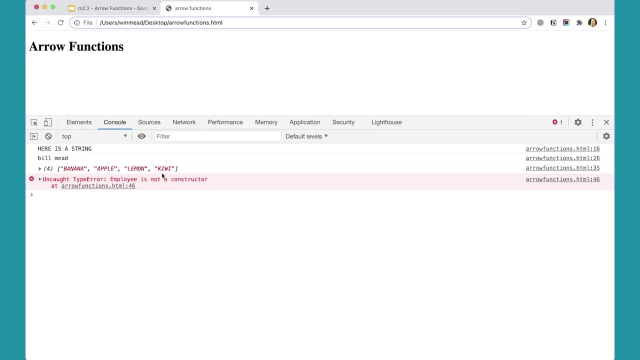 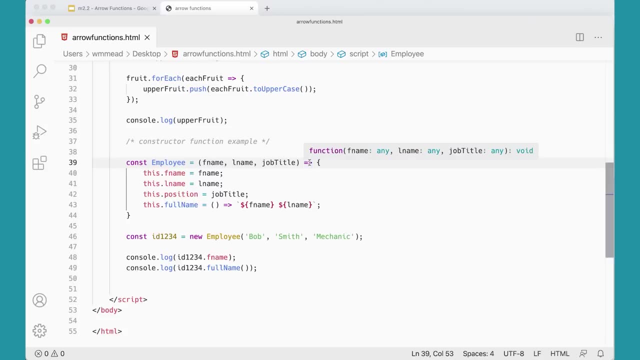 So it won't work to create constructor functions using the arrow function expressions, So we need to put that back to the way it was And then it works fine, And that has to do with the way that this keyword is scoped. In summary, 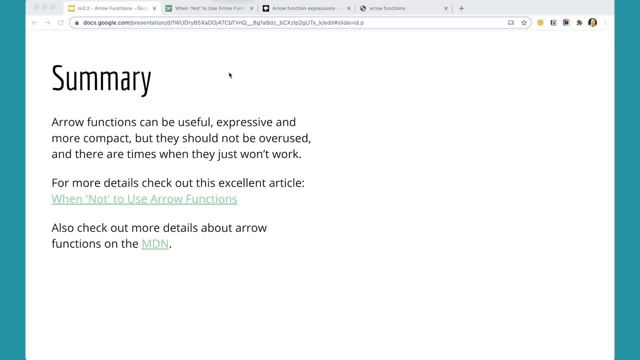 arrow functions can be very useful and very expressive and more compact, But they shouldn't be overused. There are times when they just won't work. For more details, there's a really good article here on when not to use arrow functions that you can go through for more details. 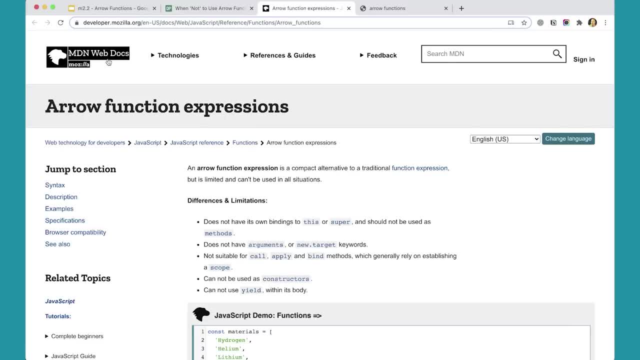 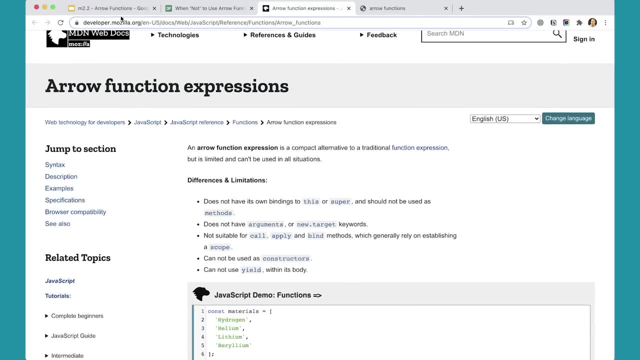 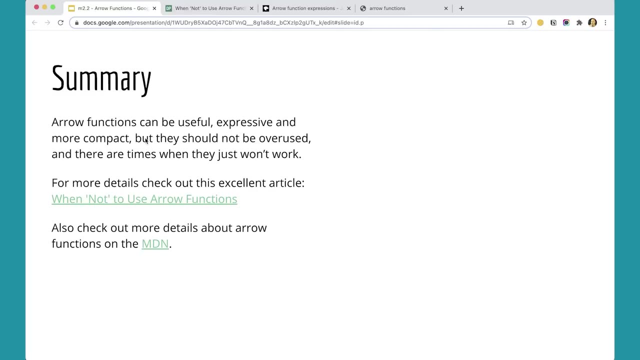 And, of course, the MDN web docs on arrow functions. expressions are really useful for examples and more details as well. So refer to those resources and I'll link them for the lesson so that you can access them easily. But there's lots to learn and lots of practice. 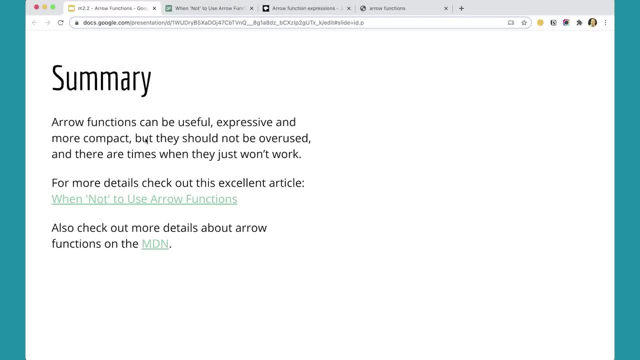 you can do with the arrow functions And I have a number of challenges that you can do. next, where you can replace functions with arrow functions and get practice and get used to the syntax. It takes some effort to get used to the syntax of arrow functions. 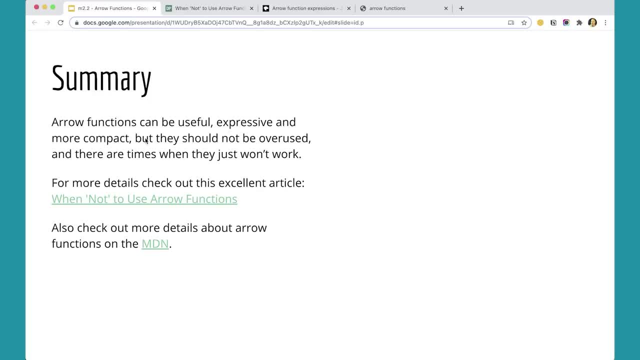 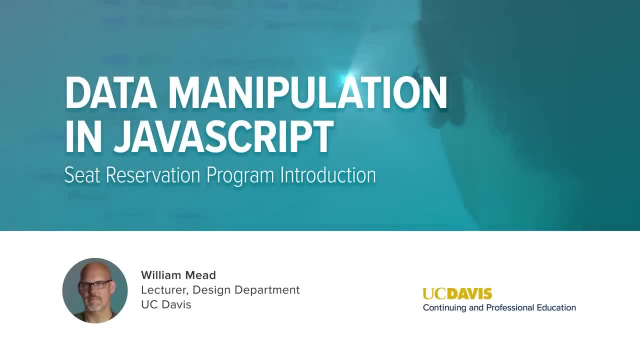 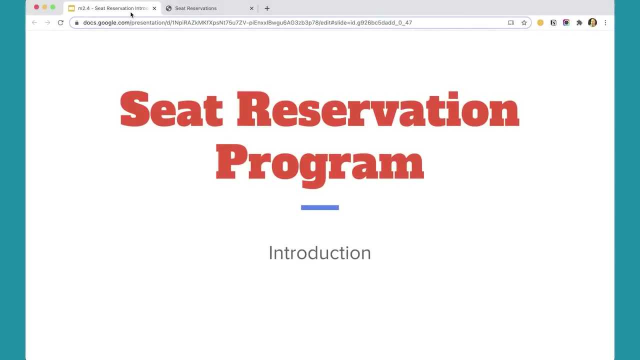 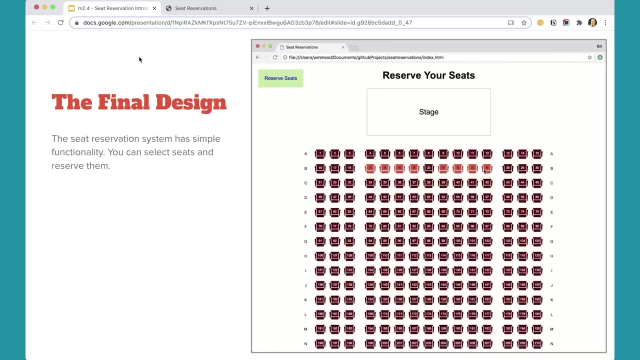 but it's worth it in the long run and you'll see them a lot around the internet in people's code. Seat Reservation Program- Introduction. Imagine for a second you're going to an event and you can purchase seats and reserve them. Not an unusual process to have. 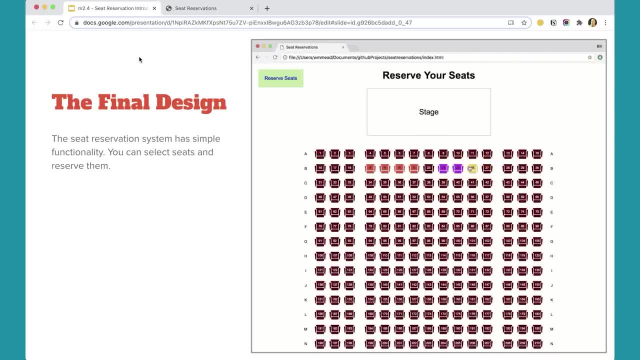 to go through if you're flying on an airplane or going to a concert or going to some other event where you can reserve the seats. So here we're going to create a system where a user can select some seats, put in their name and reserve them. 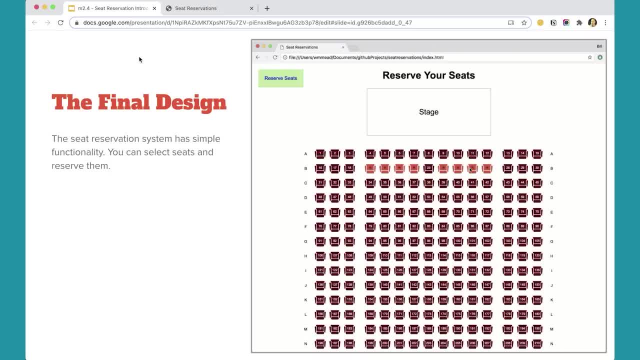 It seems fairly simple, but there's actually a lot to this project. There's a lot to consider. There's a lot of pieces to it. There are a lot of potential errors that a user could make, so we want to make sure that we can adjust for those errors as 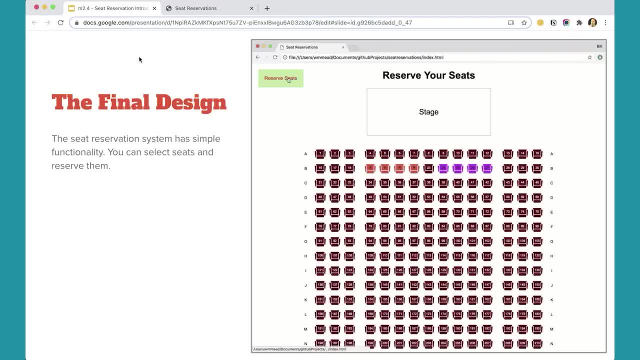 well, So here's the final design of what it's going to look like. when we're done, You can select the seats and then, when you're ready to reserve them, you can click a button and this form pops up that you can fill out, and then you can confirm. 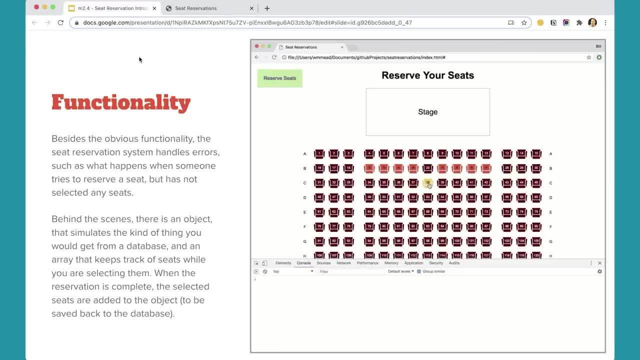 your reservation. Besides the obvious functionality, the seat reservation system needs to be able to handle errors such as what happens when someone tries to reserve a seat but hasn't selected any seats. So if they click that green button but haven't clicked any seats, what do we do? 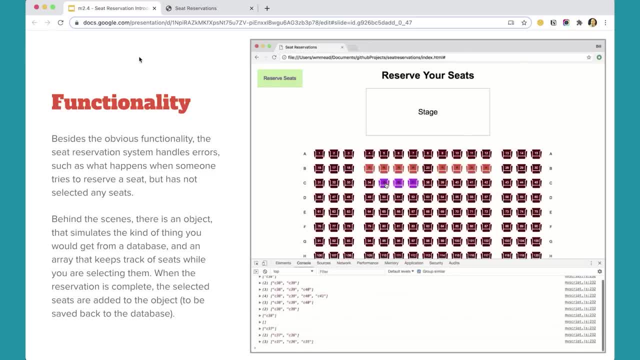 Behind the scenes also, there is an object that simulates the kind of thing you would get from a database: The seats that are already reserved. So you can't reserve seats that have been reserved by somebody else. And part of our job here is: once you've. 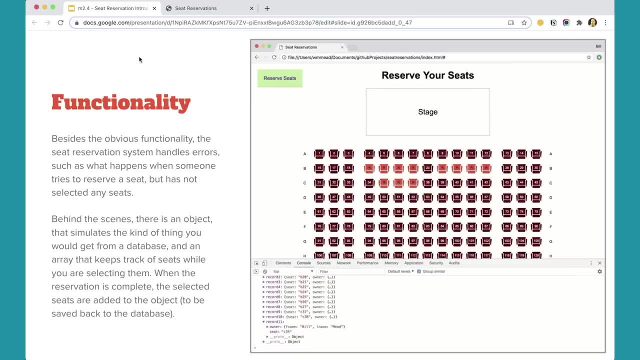 selected seats and clicked the reserve button and then filled out your name in the form. we want to be able to put those seats back into that object, which would then go back out to the database. We're not going to have an actual database for this, but just think about. 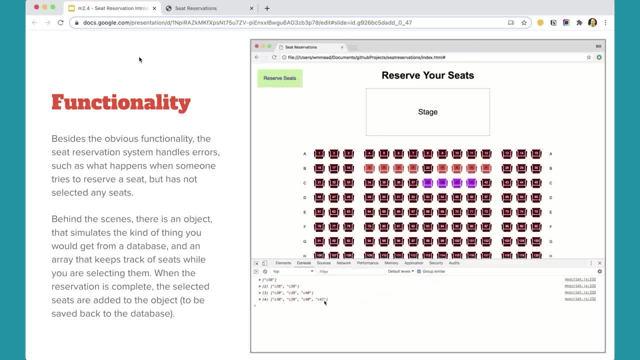 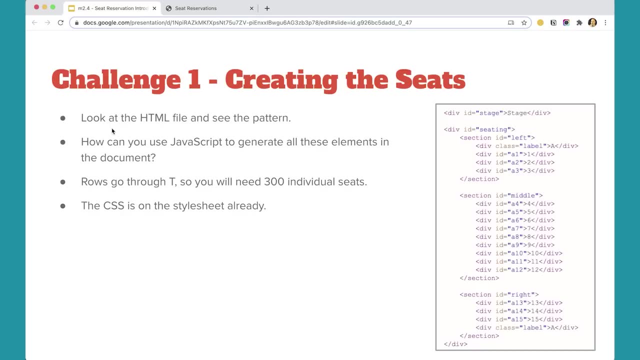 what would be necessary to put the put that data into the object so that it could go back to the database, if we had one. So your first challenge with this project is to generate seats Here. we have a lot, of, a lot of seats on the page and 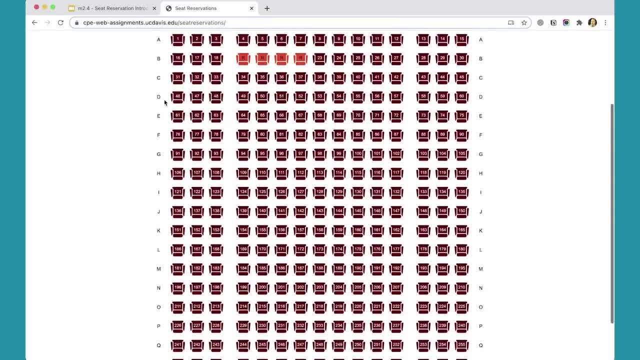 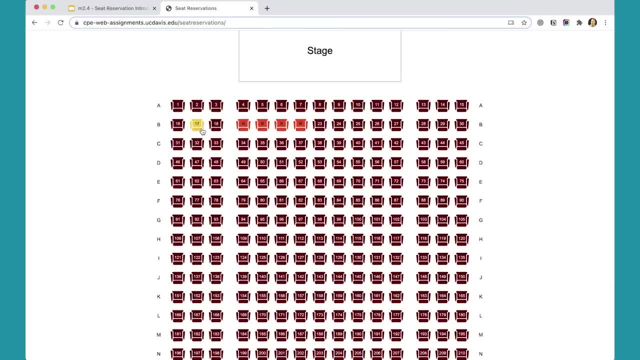 I have this final version of this here, So you can see here that I have seat number 300 and you could manually create little divs for each one of these seats. Each seat needs to have a unique ID associated with it so that I can tell this seat from that. 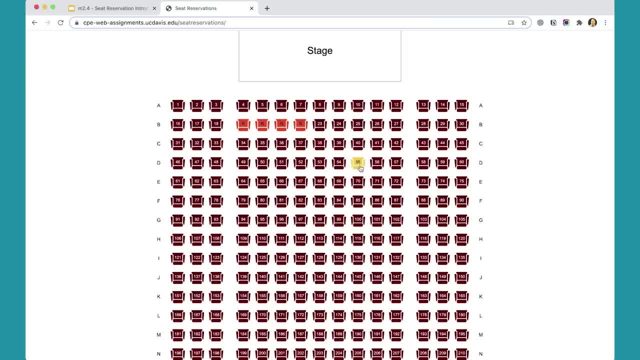 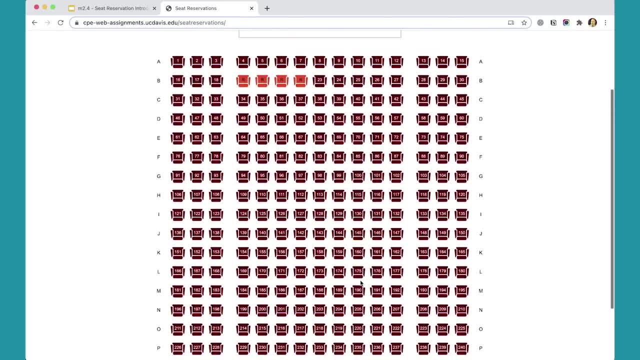 seat, And it needs to have a unique ID and a unique number inside of it, And so we need to be able to create these seats, and we could do it manually. You could create 300 divs yourself, one by one, but that's the kind of thing that 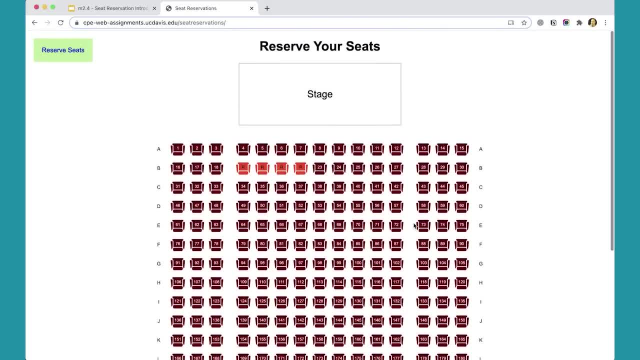 JavaScript can do, So. this is your first challenge is to do this, But also, while we're at it, think about what else is this going to need. Really think about the planning and sort of what you're going to need for this particular project. 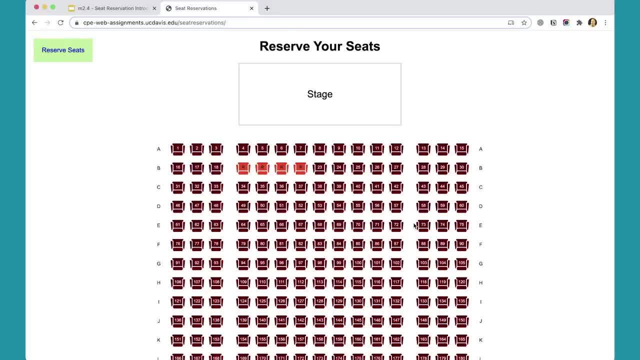 But I think it will help to take it step by step, And the first step is to create all of the seats, And we're not going to put these little graphics on it to start with. They'll just be squares We're just going to make. 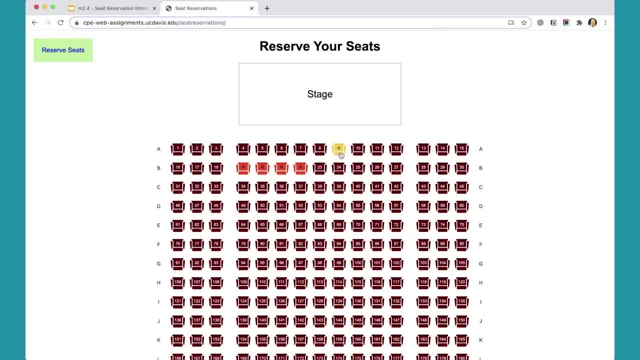 little squares that you can click on, with a number in them, And at the end, if you want the graphics, they're in the start files and you can just pop them in as background images. Just a little SVG that I created for the different. 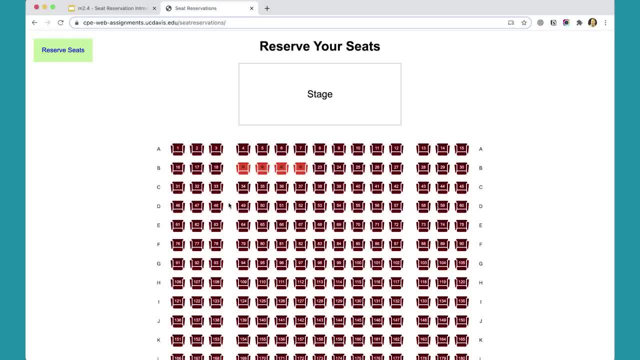 chairs here, But we can put them in the background. But to start with they're just little square divs and they're going to go on the page and we need 300 of them, All with unique IDs It's going to have. 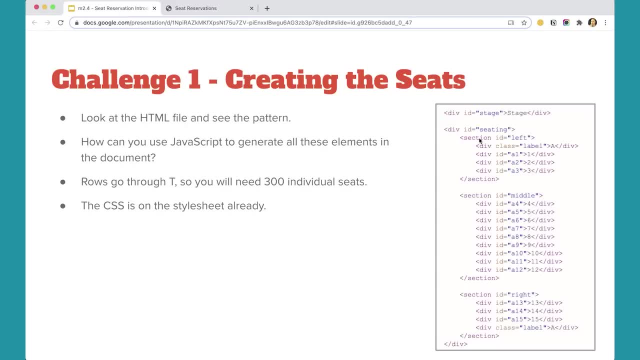 this kind of structure And the start file includes this structure for the first row, But you want to generate this structure for all of the rows. You want to have a section for the left that's going to have all of the seats on the left side, A section for. 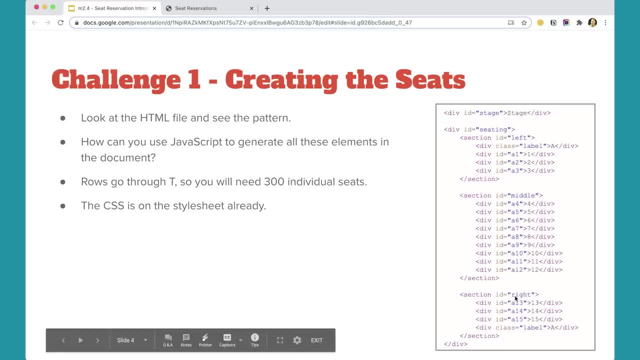 the middle. that's going to have all the seats in the middle section And a section on the right. So you're going to generate these divs that are inside these sections and figure out how to get the numbering right. That's what you need. 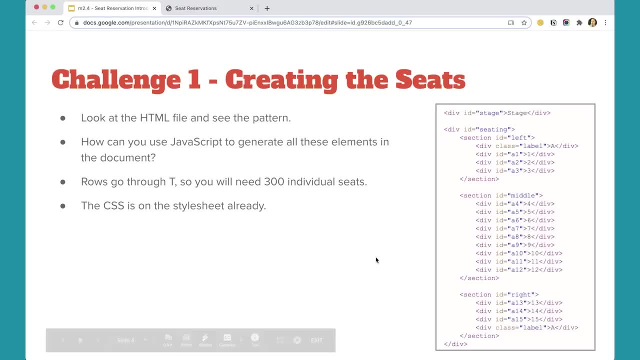 to do. That's the first challenge. Luckily, all of the CSS is done. It's already on the style sheet. You shouldn't need to touch anything in terms of CSS. So you need rows A through T and see if you can do that. See if you can. 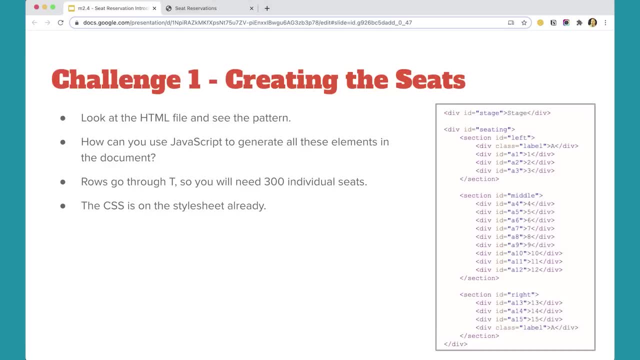 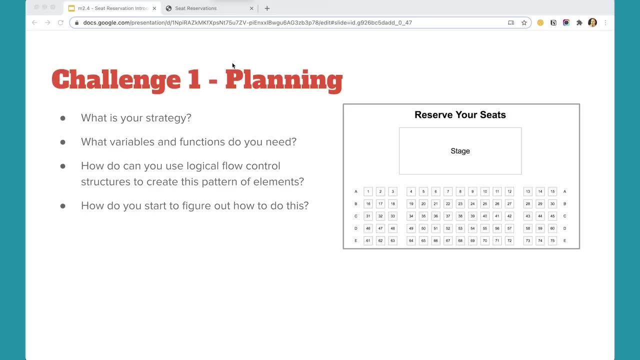 solve that challenge. To help you think about this challenge, plan it out. What's your strategy? What do you think you should do? What's the strategy for creating these and getting the numbering right as you go from section to section? What variables and 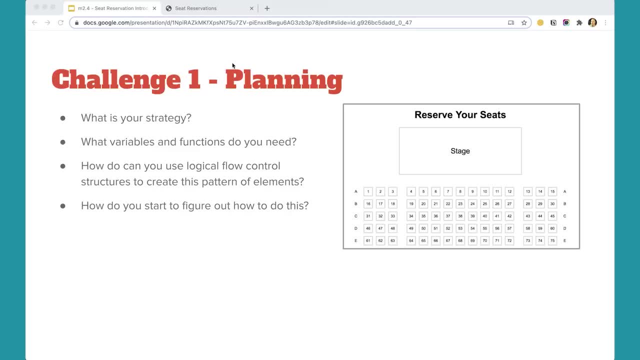 functions do you think you'll need in order to do it? How can you use the logic flow control structures, sequence selection and loop to create the kinds of patterns that you need to create to create these elements, And how do you go about starting to figure out? 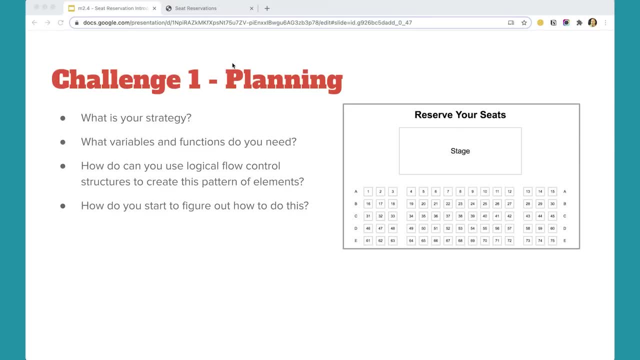 how to do this. These are the hard parts of programming- is getting over this hump of figuring out how to solve a problem. And here we're just. the simple problem we're doing is really just adding elements to the DOM, But it still takes some thought and it 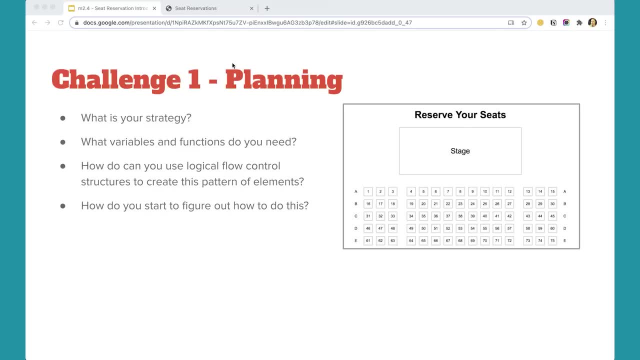 takes some practice to be able to get to the point where you can even do this much. So see if you can do it. Take on the challenge and see if you can figure out this part before going on to the next part, where I'll show you my solution. 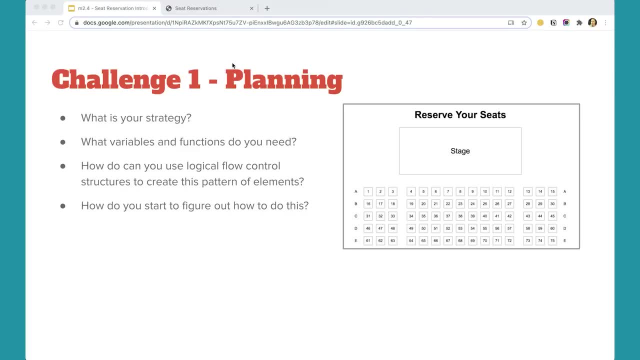 for creating the seeds, which is probably not the only solution- Certainly not the only solution for creating the seeds- But see what you can make and I look forward to popping in on the forums from time to time to see what sort of solutions you come up with. 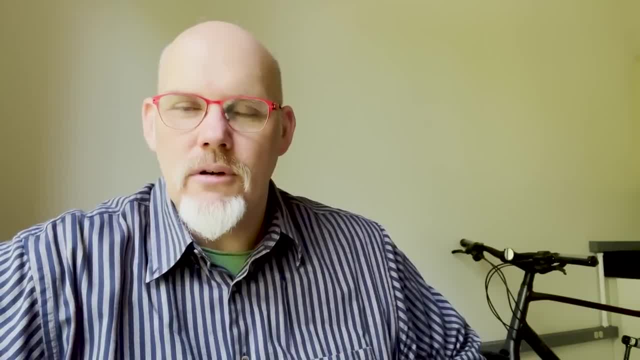 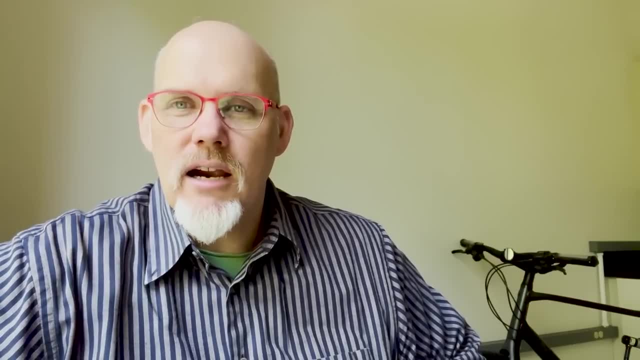 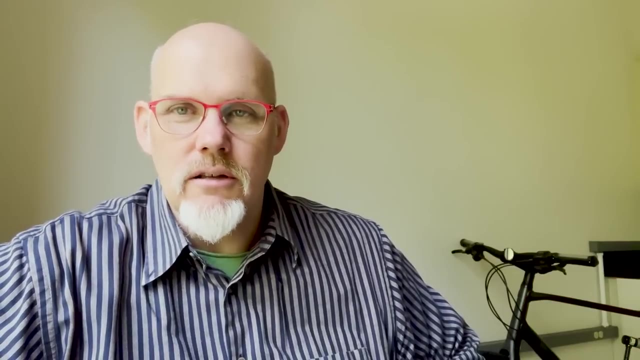 Hello and welcome to our third module in our fourth course on JavaScript. In this module we'll be building a seed reservation system. We'll spend the entire module working on this one project. It's a larger project but there's lots of small micro-challenges along the way. 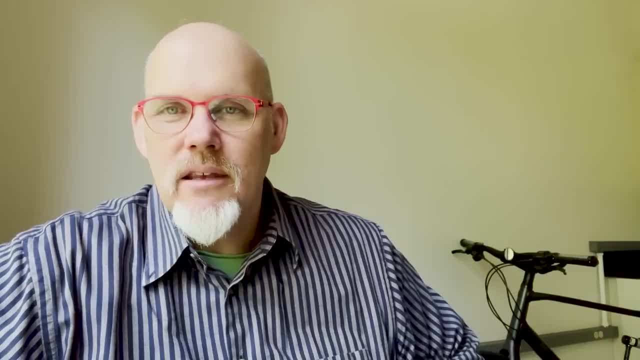 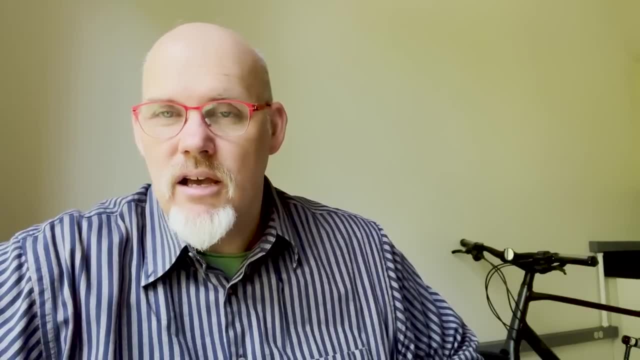 I encourage you to take those challenges and see if you can complete them before looking at my answers. But at the end you'll have a seed reservation system that shows you now how to make a small web application, And that's really powerful and very exciting. 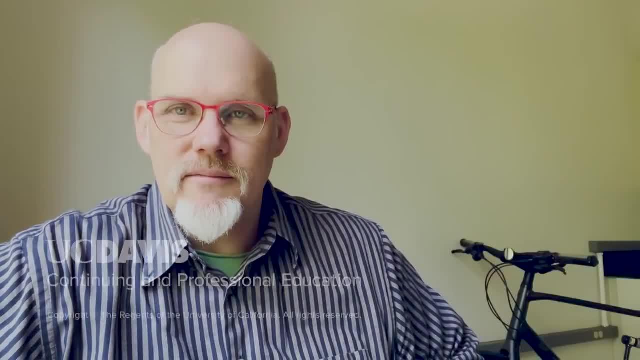 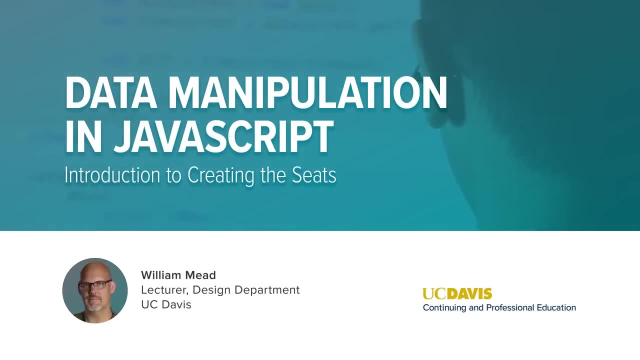 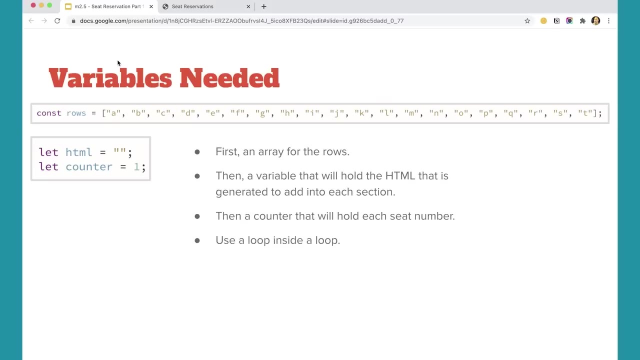 So let's buckle in and get started on it. Seed Reservation Program- Part 1: Creating the Seeds. In this part of the project, I'm going to show you the solution that I came up with for creating the seeds, And you may have come up with some. 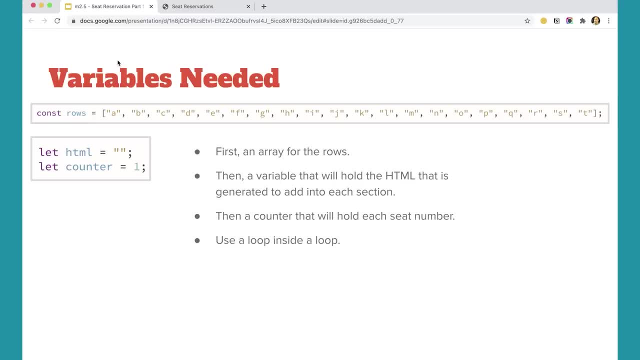 different strategies or a different way of doing it, And that's fine. There's lots of ways of doing things in JavaScript, But I'm going to show you what I came up with and you can follow along, and then we'll continue the project from here. 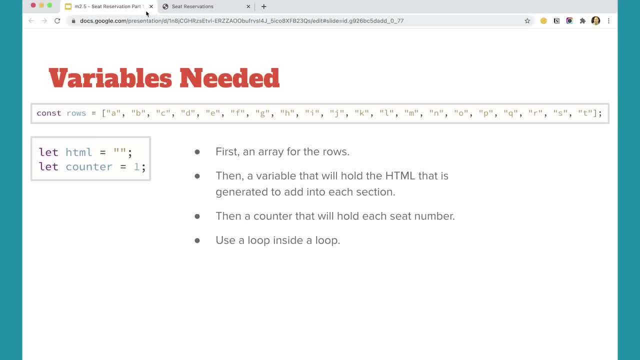 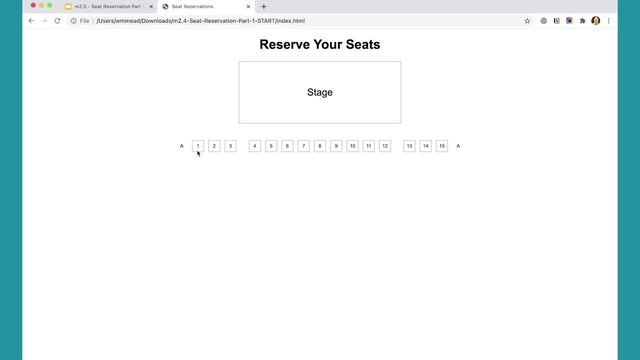 So, as you recall, we're trying to create these seeds And I have one row kind of built into the file, So there starts with a label and then we've got a section with three seeds and then a section with nine seeds and then three more seeds. 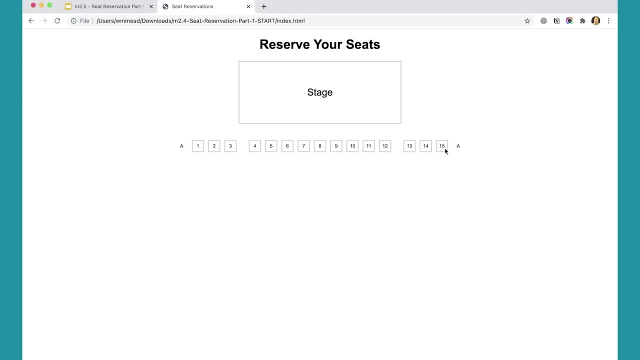 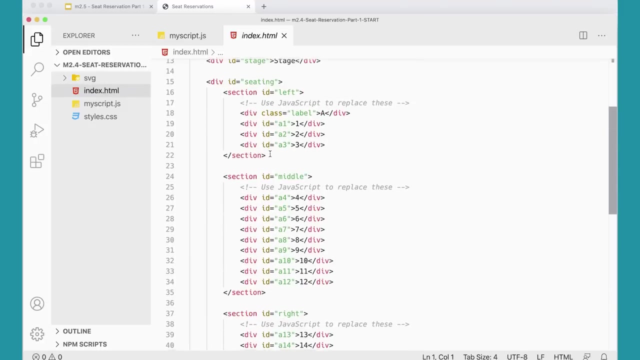 in the section on the right hand side, Followed by a label for the row on the right hand side. So that's the structure we're looking to duplicate, And I have that here in the HTML file. Ultimately, all of this will be replaced. 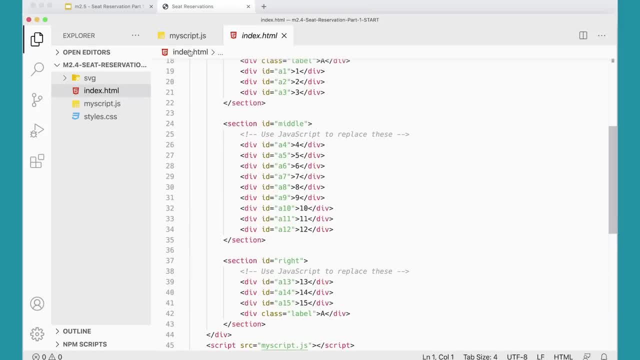 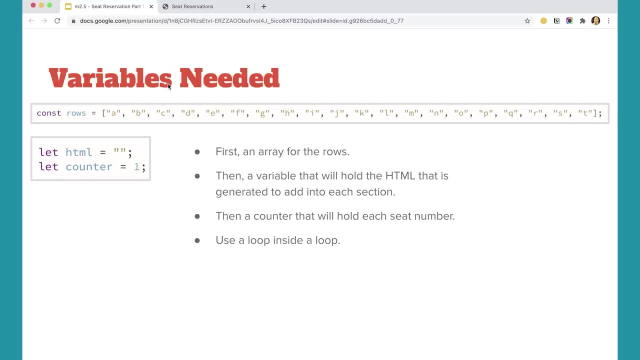 with JavaScript. So that's what we're going to be doing here in this file. My strategy is to loop through the rows, So I need an array for the rows. I'm going to loop through each row in the array And then within that row. 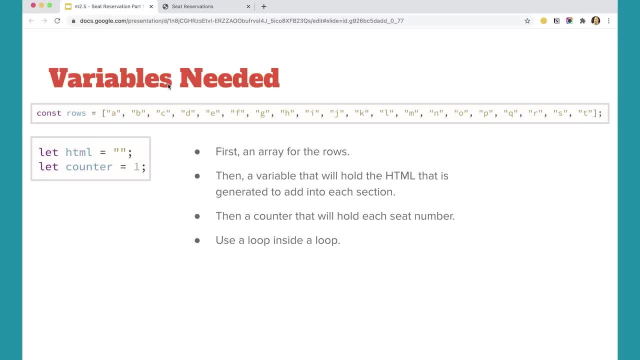 I'm going to create a variable that will hold the HTML that is generated to add that section. I'll add a counter that will hold each seat number, So we're going to need that, And then, within each row, I'm going to loop through. 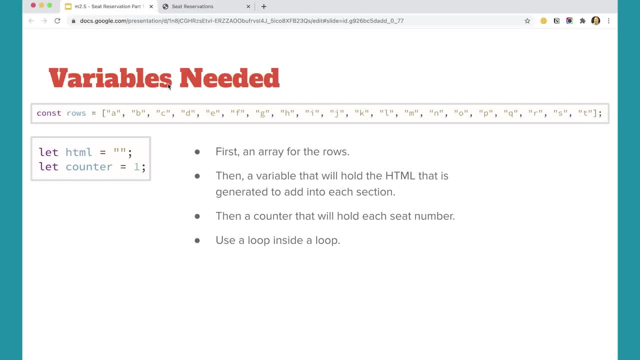 the row and create all the seats in that row. So it's going to be a loop inside of a loop, Which can always be a little bit confusing to work with if you haven't worked with loops inside of loops. So it can take a little while. 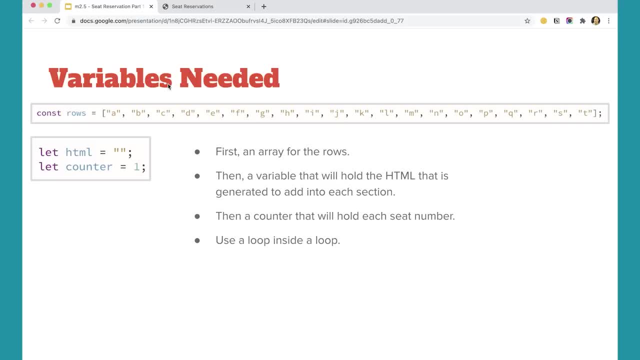 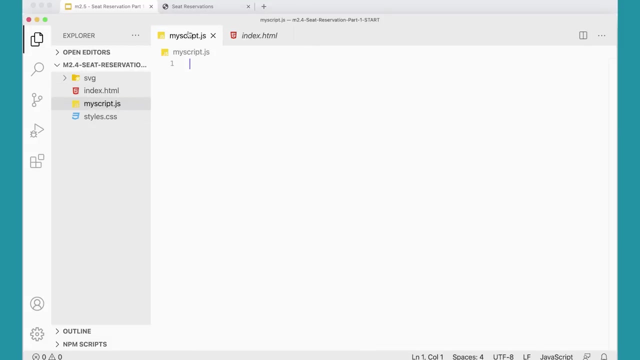 to figure that out, to wrap your brain around it, But that's the approach that I'm going to take. So the first thing we're going to need is these variables here. So I'm going to go ahead and you're going to have to type these out. 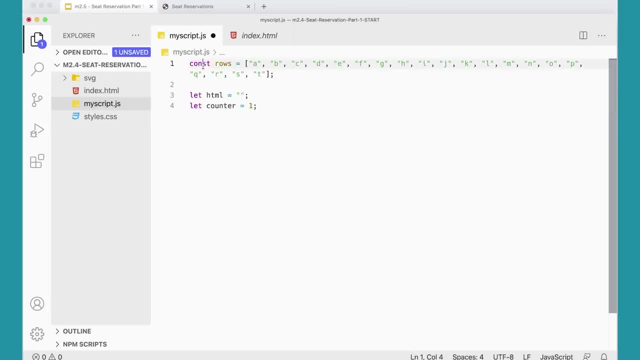 but I'm just going to paste them here on my script. So I've got an array rows with rows up to T, and then this HTML counter here is going to sort of build our HTML to add into the row, and then we've got a counter that we're going to use. 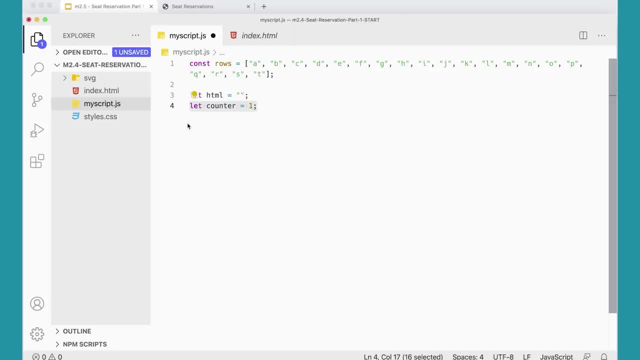 to sort of count the seats that we need and address those needs as we go along here. Okay, great, So that's working. great, Let's go and see what we need to do next. So next I'm going to use a foreach loop. 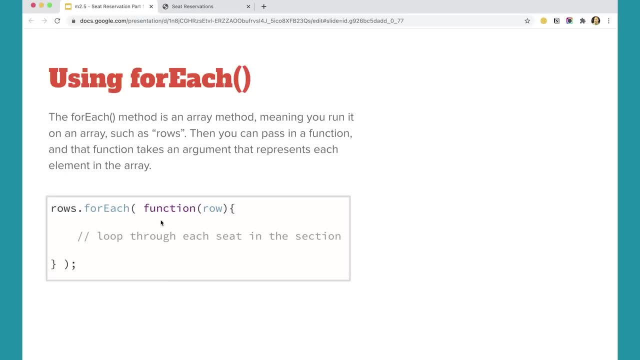 And foreach works with arrays, so we can take an array and run foreach on it. We can run a function that will pass in each row- you know, each row of the array basically- and get it going through there So we can deal with each row. 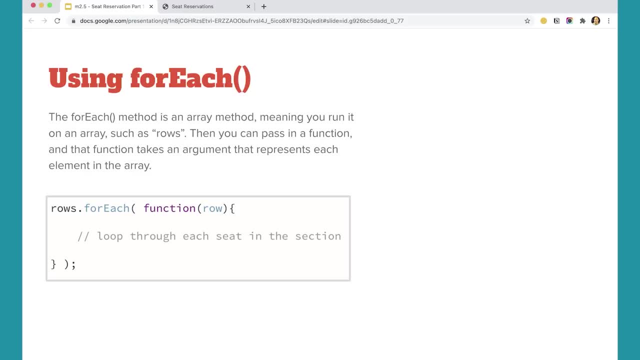 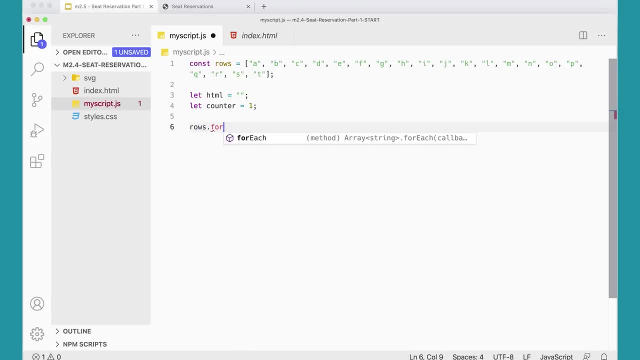 and then in there we'll loop inside each seat. So let's add this: next Rows, dot foreach. and here in here we're going to add a function And in this function we're going to pass in each row like: so: Put a semicolon at the end. 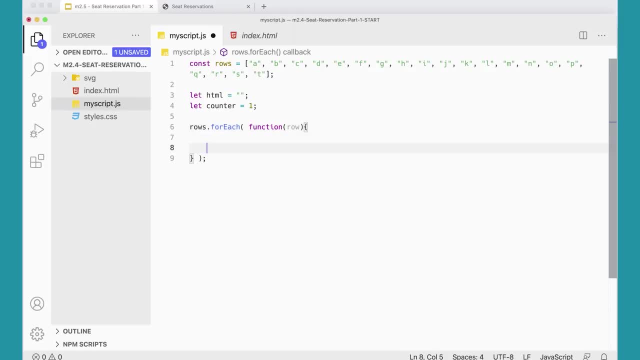 And then we're going to do everything inside these curly braces here Now. we had just said in a previous video that we could actually use arrow functions here, And I'm going to go back and refactor this at the end for the arrow functions and have you do that at that point? 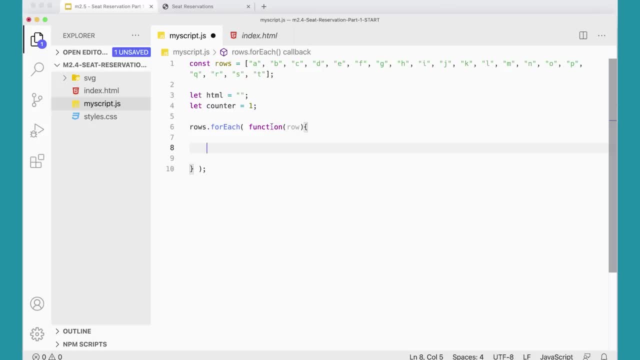 But if you wanted to, you could do it here, In which case you would remove the word function and you would put in the equals and greater. that's the end sign there, And then, because we just have one parameter, we would just pass in row. 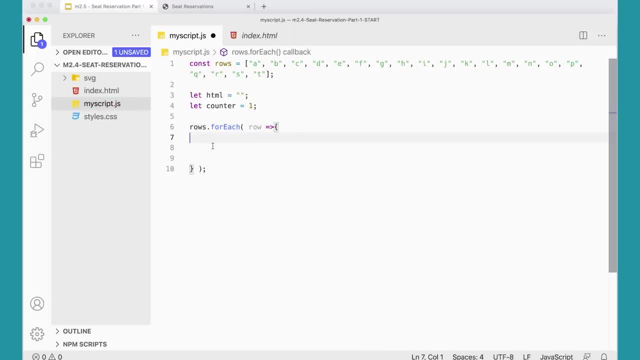 And that's all grayed out because it's unhappy because we haven't done anything with it yet. But that's fine, So you could do it that way. I'm going to leave it for now And then come back and do the arrow functions later. 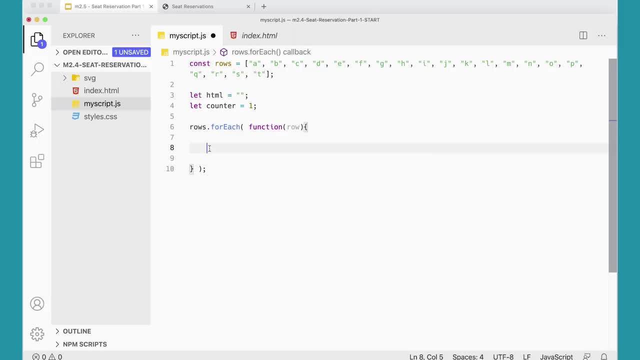 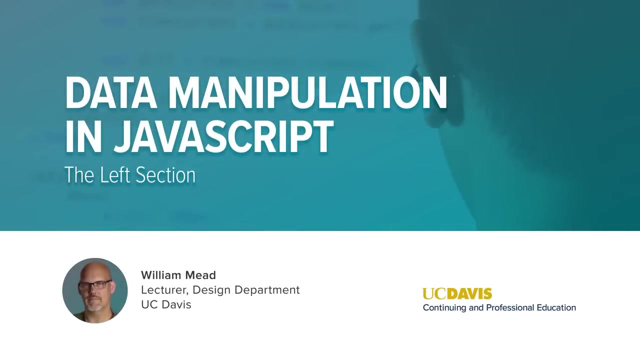 I think it's helpful to refactor for arrow functions so you can get practice writing them. I think it's helpful to see how to do it that way, But you could put them in right to start if you wanted to. Let's try to work on the left section. 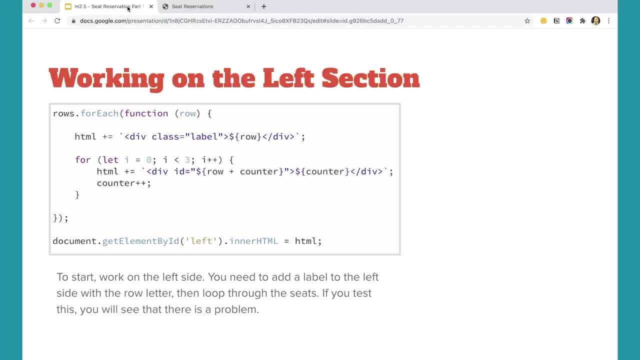 and see if we can get that working And some semblance of what we need. So what I'm going to do here is- inside my foreach is I'm going to use my HTML variable that I created and add to it. First I'm going to 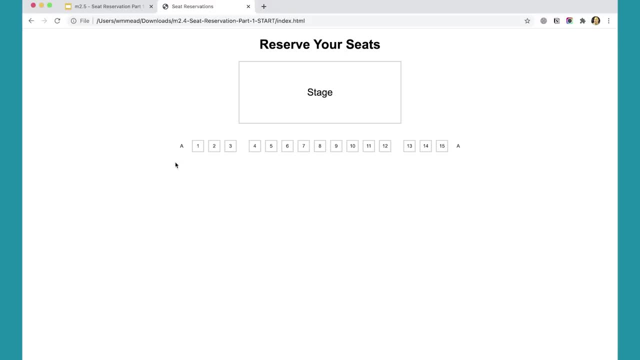 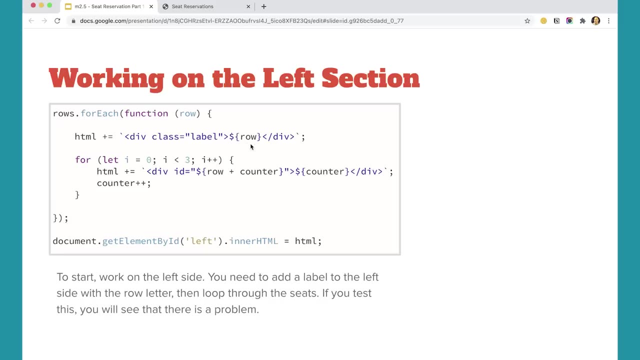 add a div to create the label. that's going to be this label here And it's got a class of label on it, And then in there I'm going to put a variable which is just the row letter, So this should create each row as we go through the. 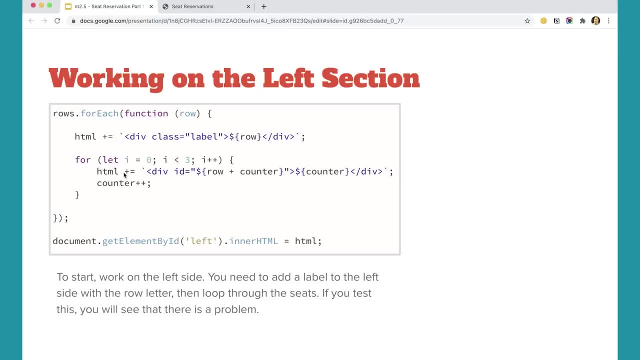 loop And then down here I'm going to make a loop that loops through and adds also to that HTML a div for each seat with the counter, And then I'll simply add that to the DOM. So let's go ahead and try that and see what we get. 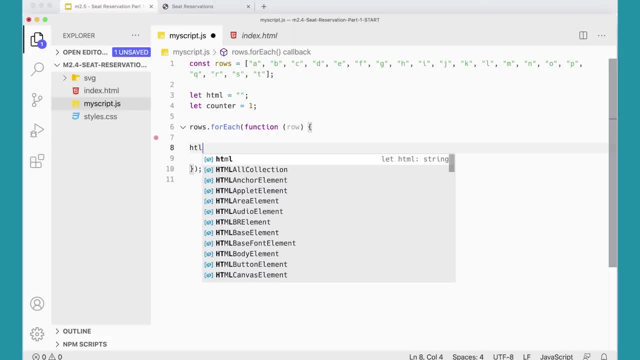 So if I come over here, I'm going to take my HTML variable and I'm going to add: I'm going to tab that in actually HTML plus equals. So we're going to add to it. I'm going to use my tick marks with a semicolon at the end. 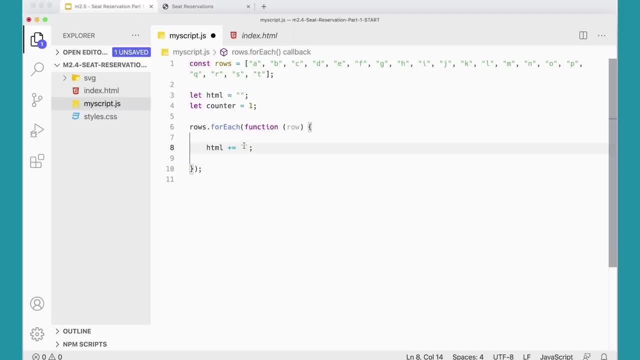 And in there I'm going to put a div which is going to open and close, And I really recommend you type this way. Get used to typing from the outside in. I know I've been saying that all along, but it's really easy to forget. 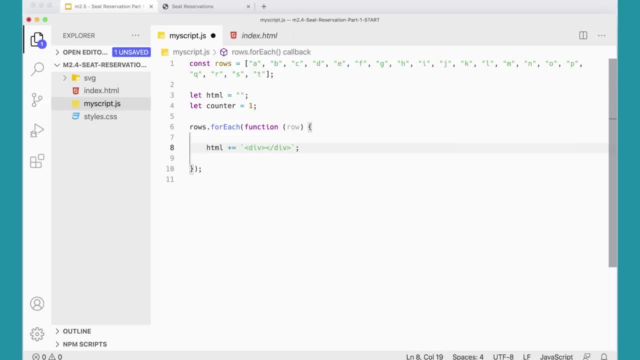 And then in here is a variable, So I'm going to do that and then that's going to be this row. So we're going to loop through each row. so the first time through this for each loop, that's going to be an A. 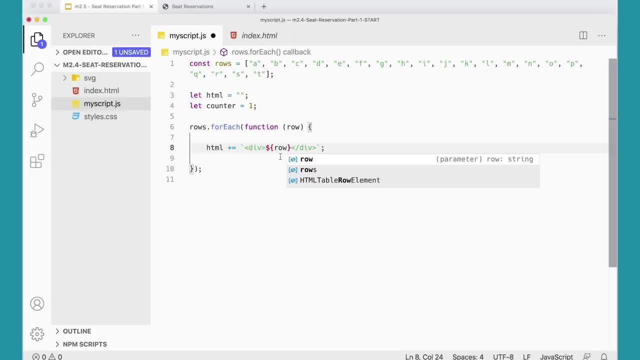 And then the second time it's going to be a B, and then the third time a C, and so on and so forth. So that will create that. and then we also need class equals quote label on this as well, to work with the styling that I have here. 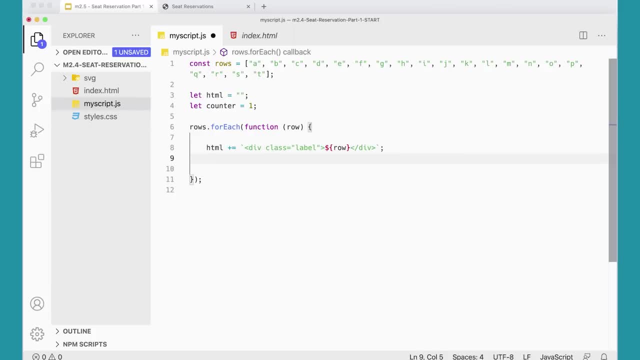 in the style sheet. And then we're going to have a forward loop, For I'm going to make another return there, For let i equals zero, while i is less than three, because we know we've got three seats- i plus, plus- and then in here. 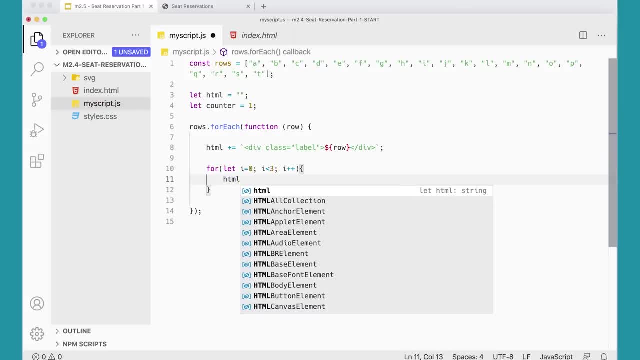 also with the HTML. I'm going to add: plus equals zero, equals my tick marks and a semicolon, and I'm going to put another div which is going to open and close and in there is going to go this variable counter. I need to do my variable. 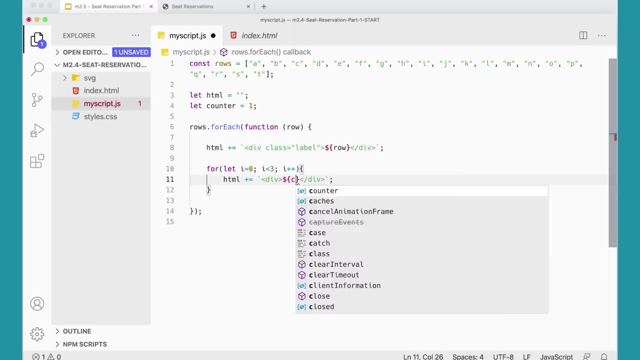 dollar sign curly braces counter and it's going to get an ID ID equals quote, quote and in that is going to be a variable dollar sign curly braces and the variable in there is going to be row. so I'll get an A plus the counter. so the first. 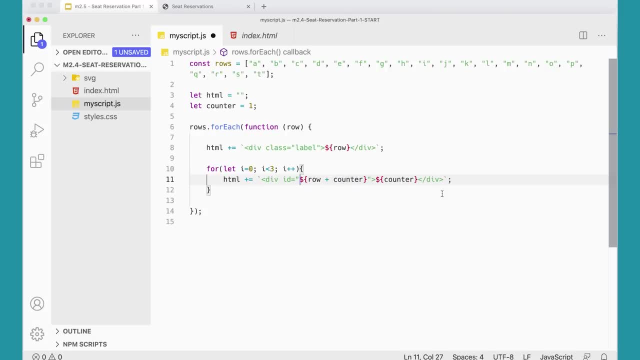 seat will be A1 and then A2, and so on and so forth, and then we have to increment the counter in here. So I'm going to do counter plus plus. so what that should do is: I've got a loop of three, so it should create. 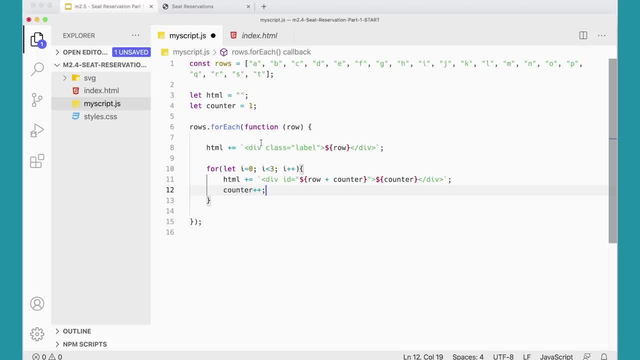 a label, then three seats and then a label and then three seats and then a label and three seats until it's done with all of the rows down through T and I should be getting, and that counter is going to keep going up the whole time, so I'll get. 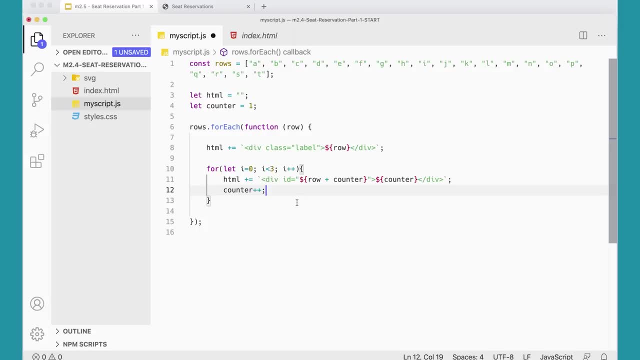 one, two, three in the first row and four, five, six in the next row, and that's not going to be right for our project, but at least it's something to get started with, and then down here we just need to add this to the DOM. so after my foreach, 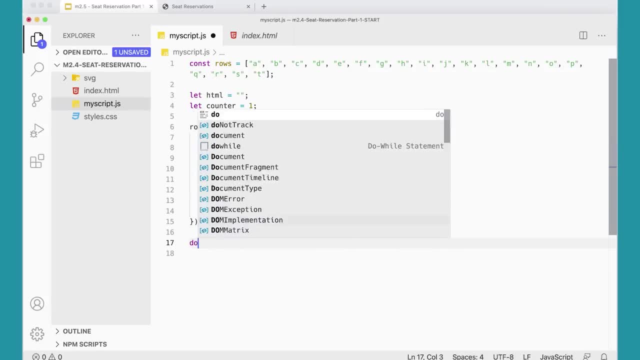 I'm going to put document dot get element by ID and I need left, I need the left side and I do dot inner HTML and I'm going to put the HTML in there that I've created. okay, great, let's see if this works. I'm going to come over here to 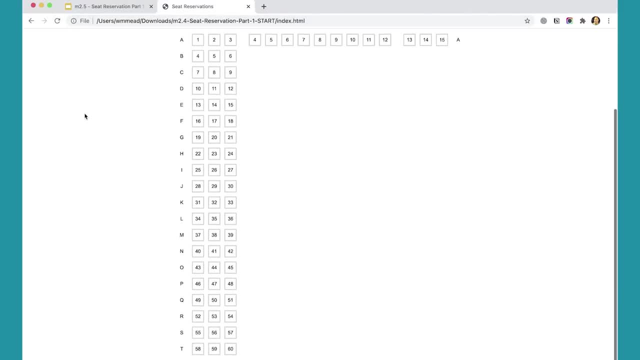 my page and refresh and look at that I've created sixty divs all at once here. now you'll notice the numbering is not correct for what we need for our project, because I've got one, two, three and then the middle section would be four through twelve. 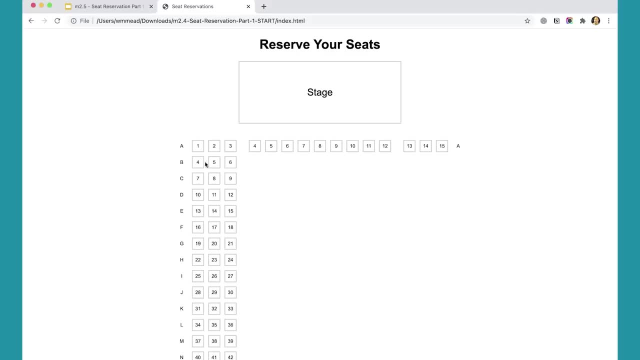 and then the right section would be thirteen, fourteen and fifteen, but now I've got four over here again. now there are different ways of approaching this. you could think of the venue as having different labels for different sections and having all the numbering for the sections work like this. 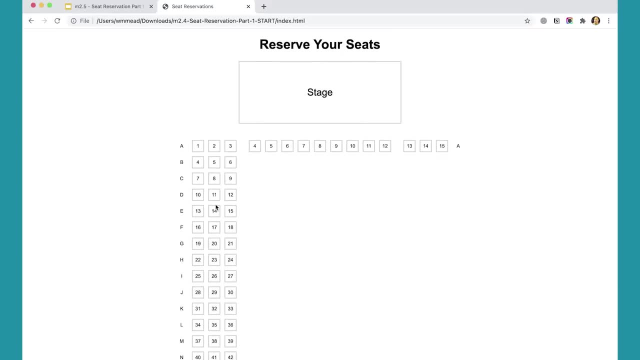 that would be one way of doing it, or another way of doing it would be to have one through fifteen for row A and then one through fifteen for row B and then one through fifteen for row C. that would be another way of doing it. but what I asked specifically, 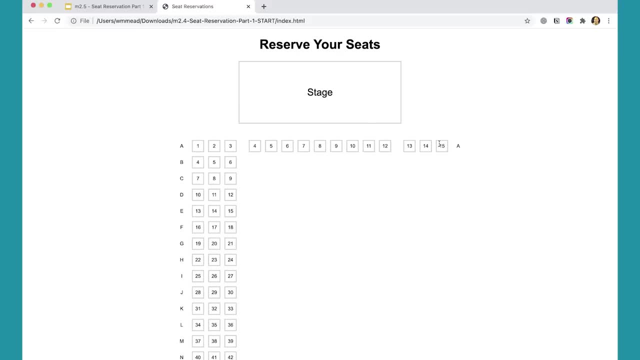 for was to count them up so that that goes to fifteen, and then this one should be sixteen, seventeen and eighteen, and then these would go on over to thirty, and then we would start with thirty one, thirty two, thirty three here. that's what I asked for specifically. 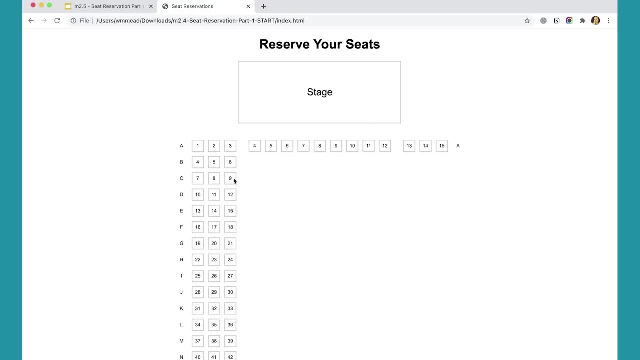 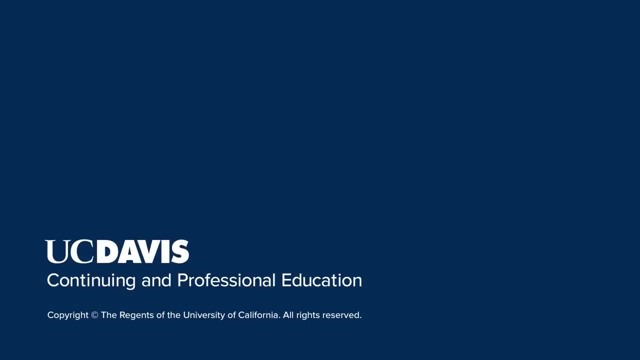 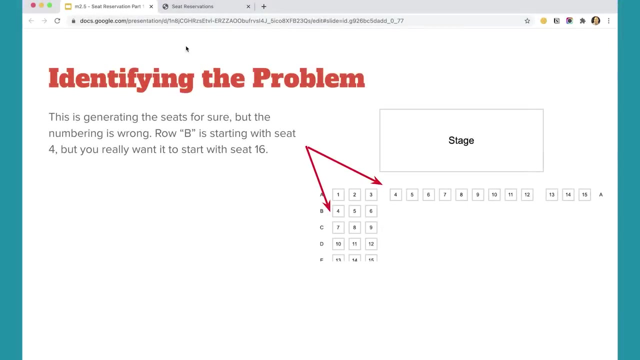 so maybe this venue wants that particular numbering system for some specific business reason. that's the way they number their seats, so we need to mimic that. so that will be the next problem to solve. how could we fix that problem? in the last video we identified this problem of the numbering of the. 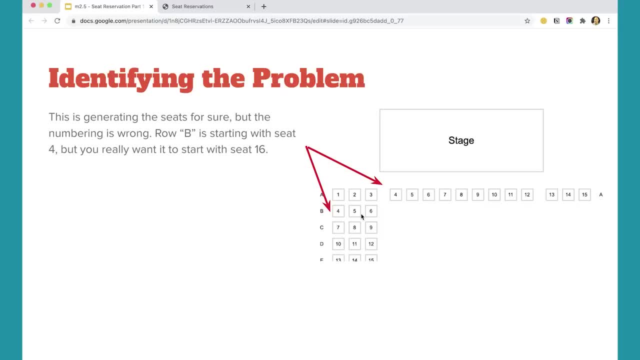 seats as we go through here, and that's great. so now we can try to fix that problem. I don't know if you tried to come up with a solution or thought of a solution, but here's a solution I came up with. I could take the counter. 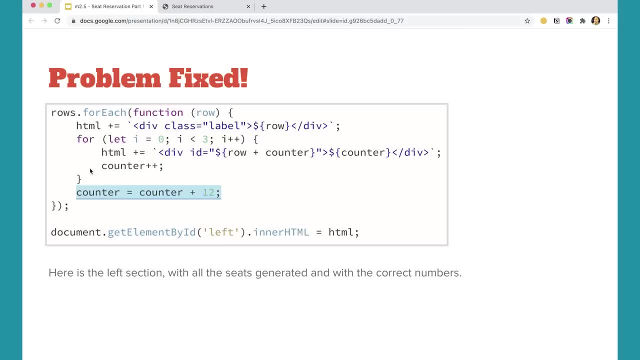 after my for loop. so it's going to count three things, and then I could take that counter and increment it by twelve before the next iteration of the for each loop, and that will actually solve that problem. so let's give that a try. come over here and 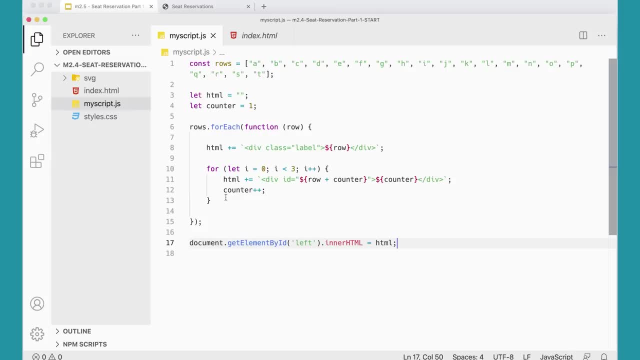 outside of this loop. so it's going to count one, two, three, and when it finishes those before it goes on to the next row, I'm going to take counter and make it equal to counter plus twelve, like that, and that will then say: okay, so now I do one, two, three. 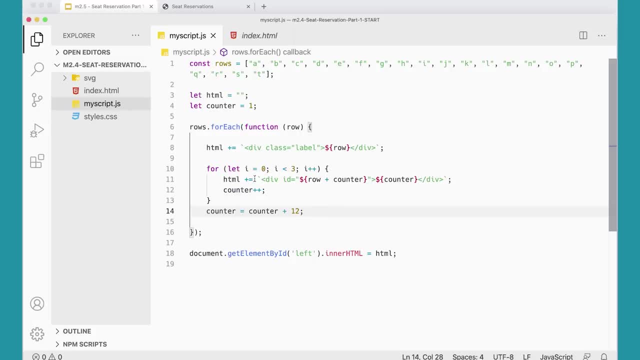 then I'm going to add twelve to counter, and the next time for row. for row b, so that's for row a. when it finishes row a, for row b, it's going to add twelve to that counter after it did three. so then the next one when it gets to. 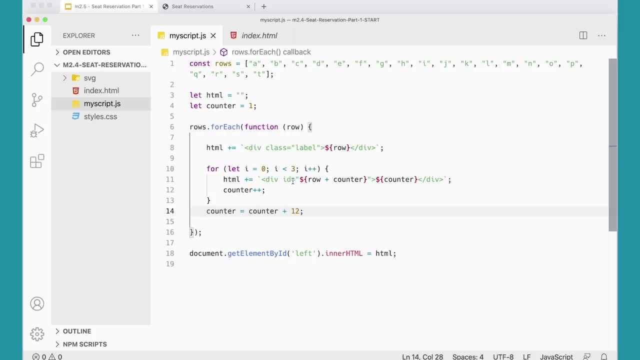 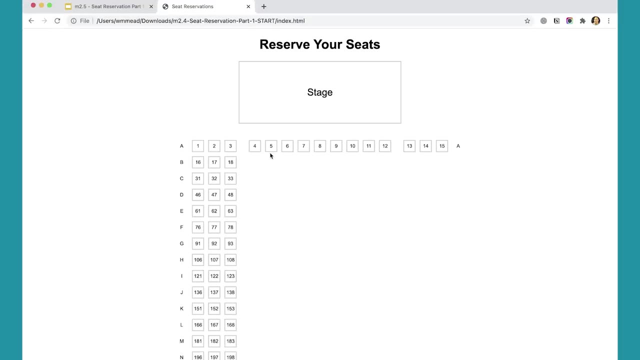 row b will be sixteen, seventeen and eighteen here. so let's test it and see if that works. and there we go. so we're getting all of the right numbers here. so fifteen, sixteen, seventeen and eighteen, and then we get over here. that will be thirty by the time we get there. 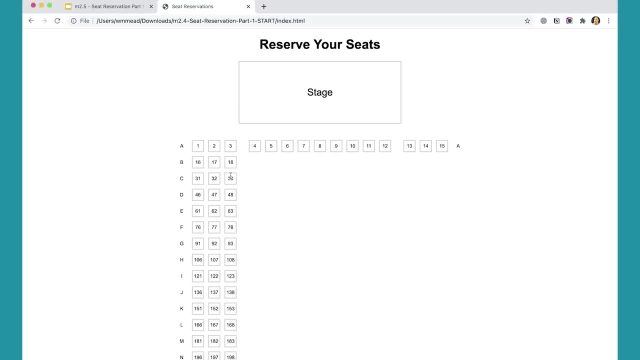 when we come back. so this should be thirty one, thirty two and thirty three, so on and so forth, with fifteen seats per row. that's how that would work out great. so that's working great. so now we could we have sort of a template to work on. 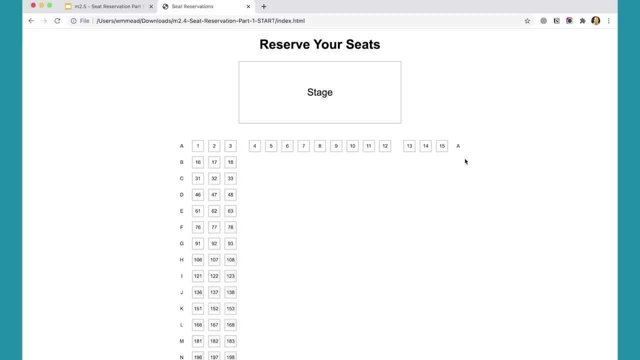 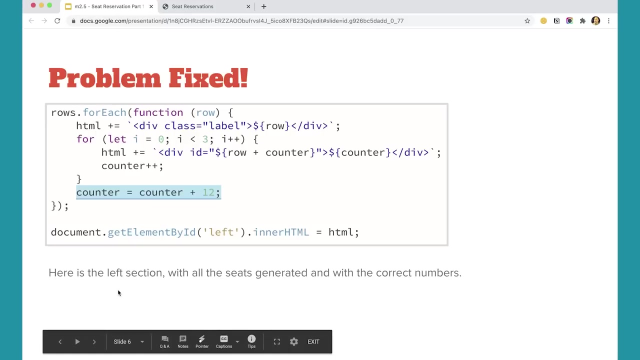 the left side. we could do the right side, which is the same thing. it's just reversed. we're doing the three seats and then the label, and we need to add to the counter before we do the three seats. so that shouldn't be too hard to do, because it's very similar to. 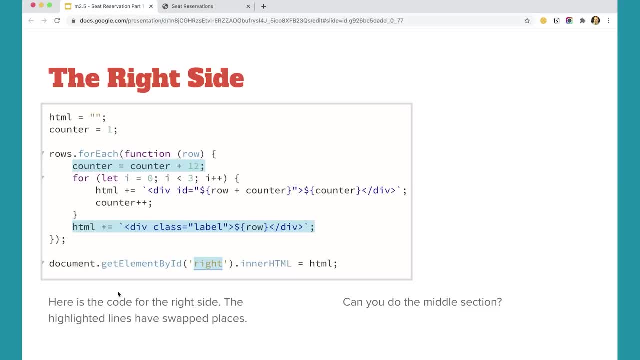 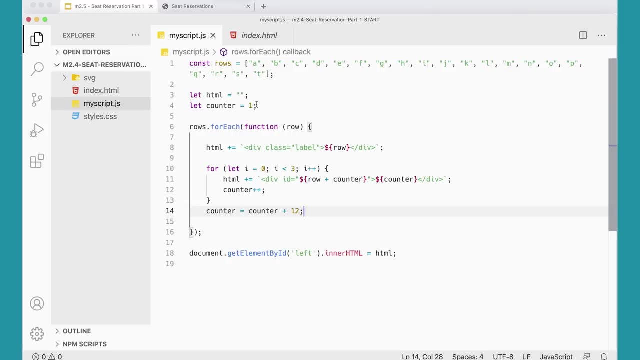 what we have. so here's what I have for the right side. so let's go ahead and add that in here. I'm going to need the these two variables again. I can leave the rows- that's going to stay the same, but I'm going to need these. 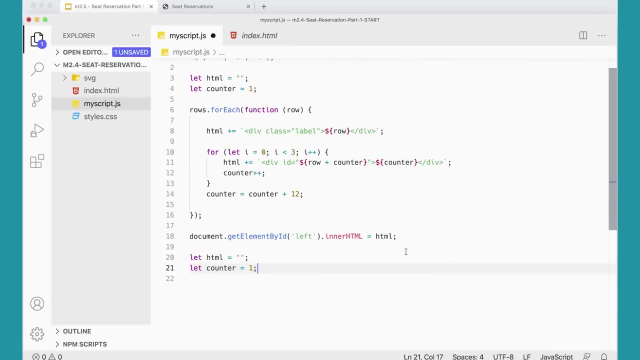 two variables again and we'll refactor this all down. but- and another thing to notice is that I knew up front that this wasn't going to be right for the numbering. but you have to start somewhere. so try to get something working and then from there you can. 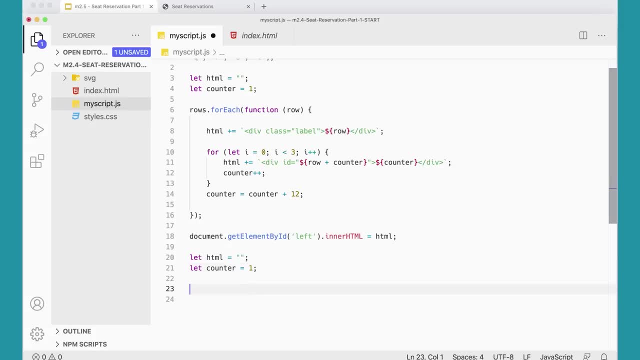 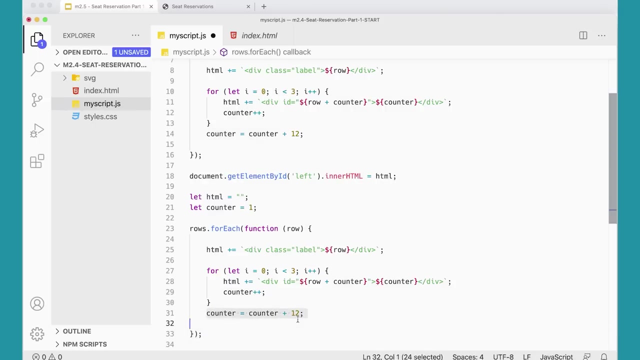 see what you need to do to fix it, to get it to work exactly the way you want to. so I'm going to just copy this and paste it down here. but instead of having the counter at the end, I'm going to add 12 seats to the beginning. 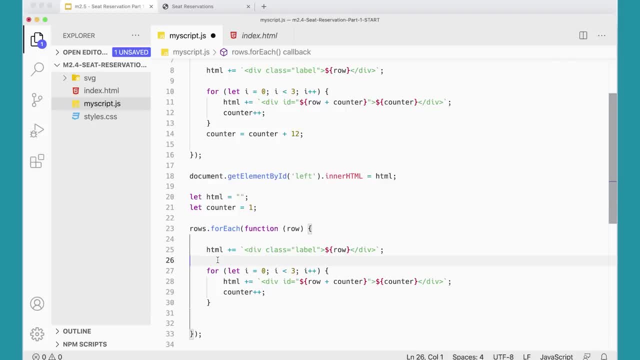 so I'm going to take that out and stick it here, because I want to add 12 seats and then start with my number for the counter. so it would be. so I would add 12 seats, so this first one would be 13 and then the second time through it would be. 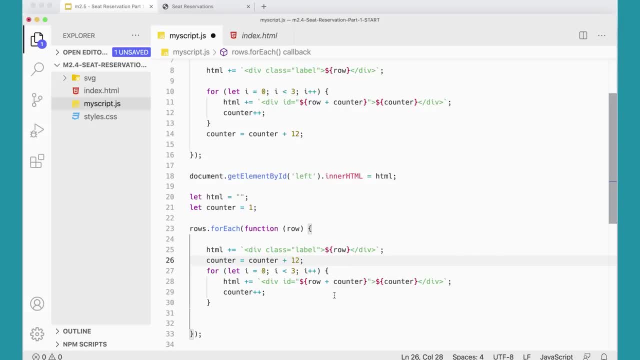 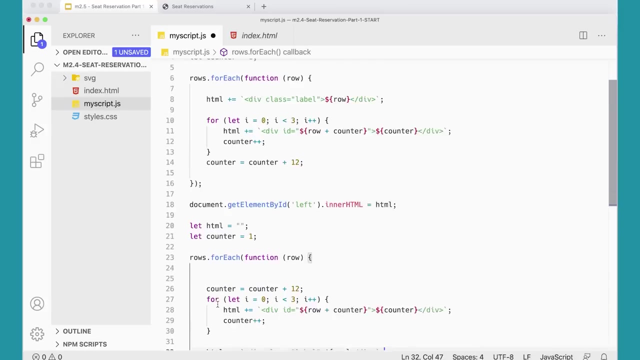 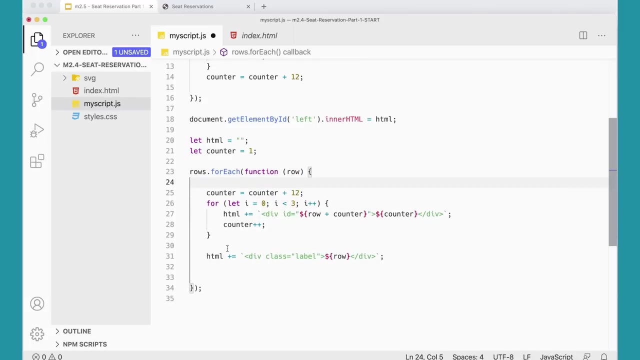 14 and then 15. yeah, as that works. also, I need to move this down to the bottom because I want to put the label at the end, correct? I want to do the seats first and then have the label to get to the right side over here. 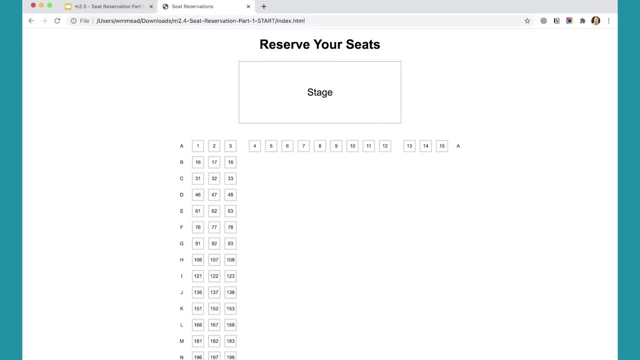 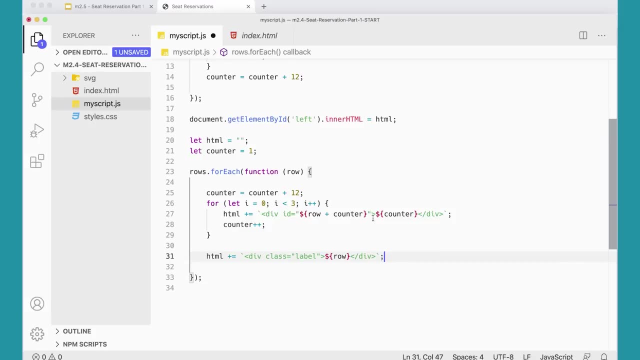 the seats first and then the label, if that makes sense. alright, so we put that in there and and that should take care of the right side. I just need this piece here, copy that and stick it down here and change this to right, save that, and let's go take a look and see. 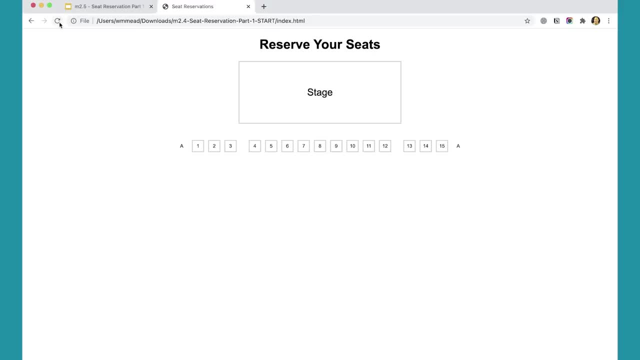 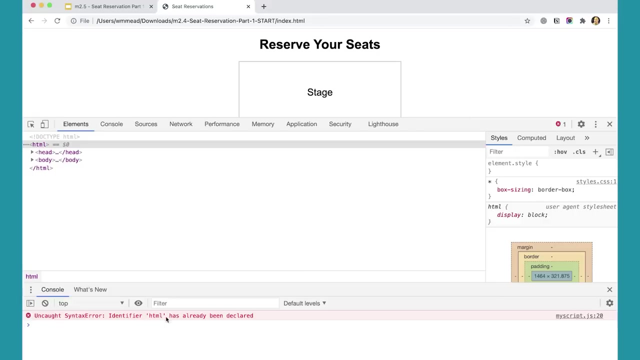 if that actually worked, if I did that right. oops, I must have a mistake somewhere. so this is very typical. of course, you probably have a syntax error. inspect and I can see I have a syntax error here. identifier html has already been declared. oh, I see what I've done. 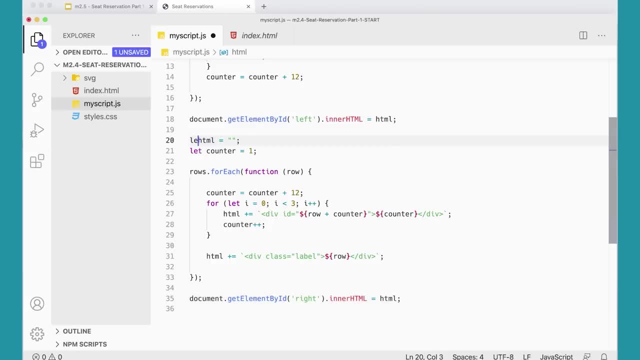 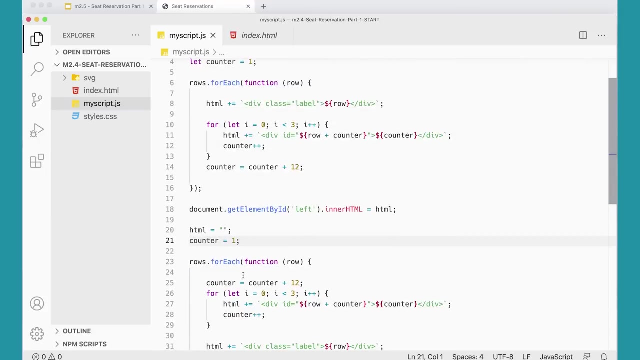 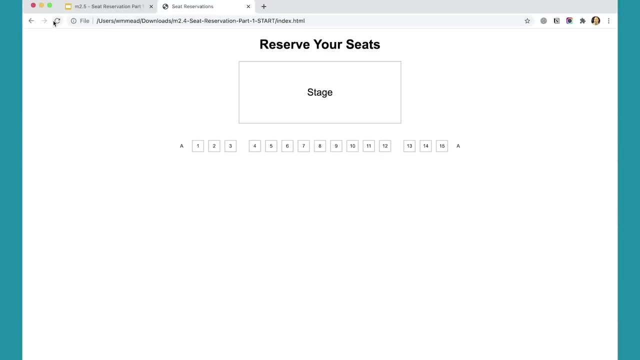 I can't say: let html here. I can just set html encounter back here. there we go, because I had already defined it up here. I can't redefine it like that. ok, great, so let's go back and test this again. close my inspector and there we go. 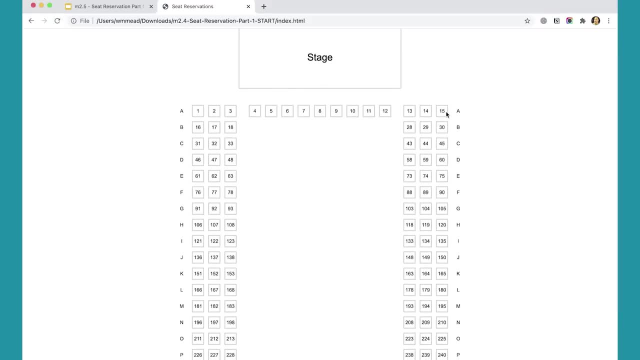 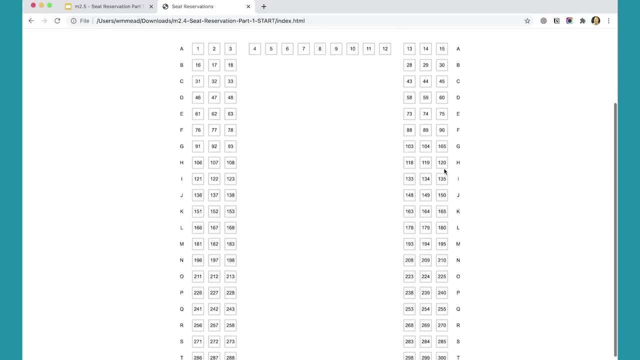 so I've got 1,, 2,, 3, down here I've got 13,, 14,, 15, this is 16,, 17 and 18, and then over here I've got 28,, 29 and 30. so that's working great all the way down. 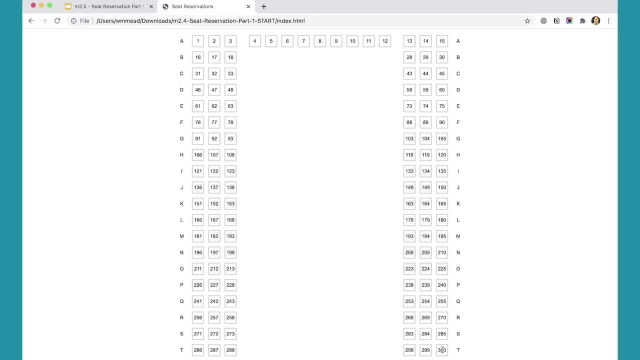 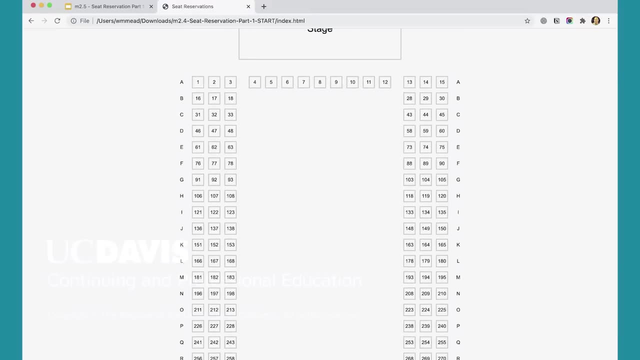 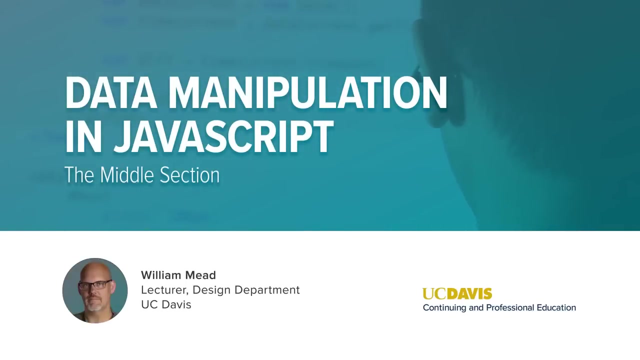 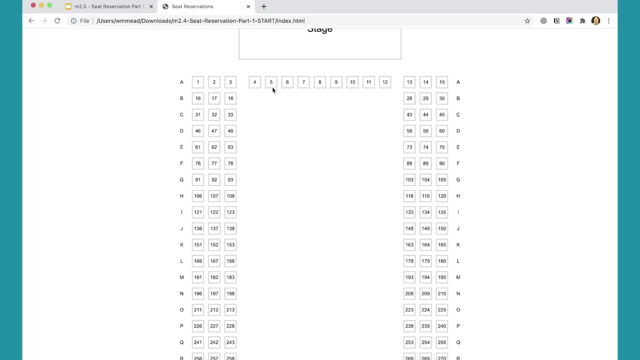 to my very last square, which is square number 300, and in the next video we'll take care of the center part of the stage. in the previous video we figured out how to get the right side to display properly, and we have that working here, so that's great. 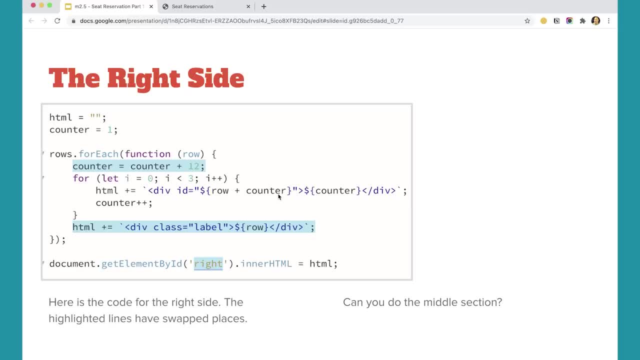 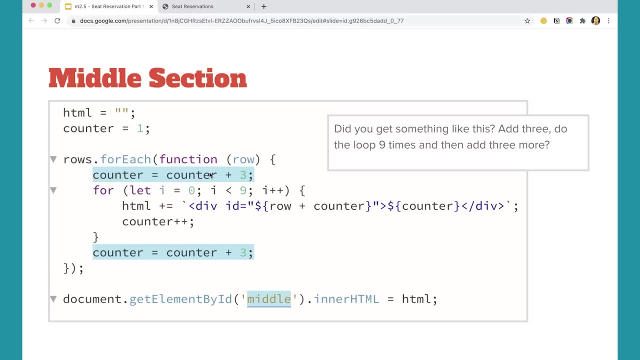 now we need to just do the middle, and for the middle you can imagine that it's just a slight variation on what we've done here. we need to add 3 seats for the left side and then do the counter for 9 seats, because we're going to have 9 seats in the middle. 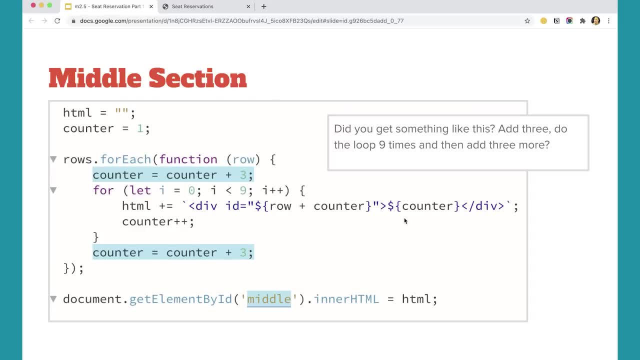 and then we'll add those seats in there, and then we need to add 3 seats for the right side at the end of the foreach and then we can just add this to the middle. so that shouldn't be too difficult to do, based on what we already. 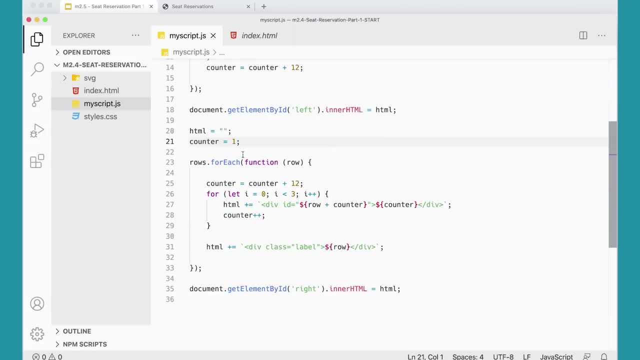 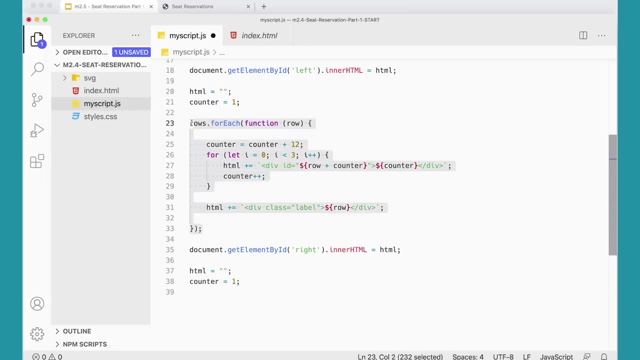 have. I'm going to come in here and I'm going to start by. we're going to need to set these again, so I'm going to copy those and paste them down here, and then I'm going to copy this whole loop here. copy that and paste it down here. 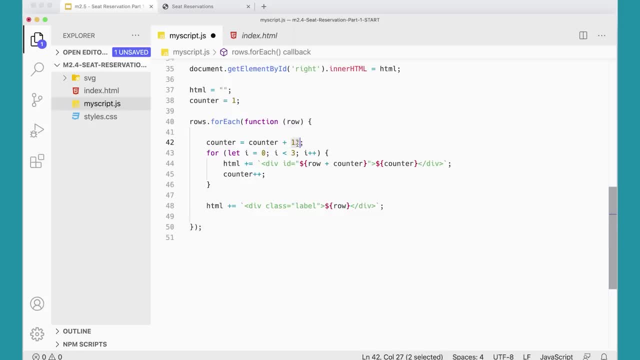 foreach function row, but here I want to add 3, and then at the end I want to add 3 more. so I'm going to copy that and paste it down here. so we have 3 more there. we don't need the label at all for this. 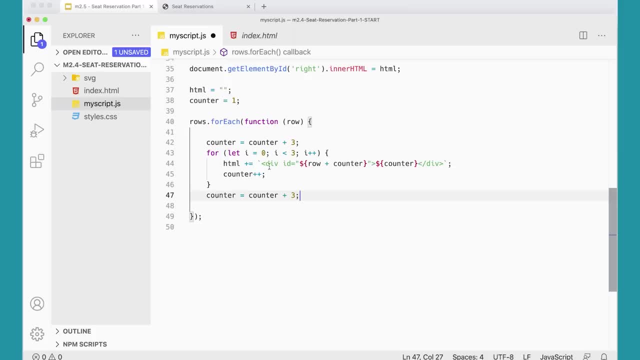 middle part, so we can just get rid of that. that kind of makes it a little bit easier. and then in here we're going to put in 9 seats. so I'm going to change that to a 9 and that will put in 9 seats. 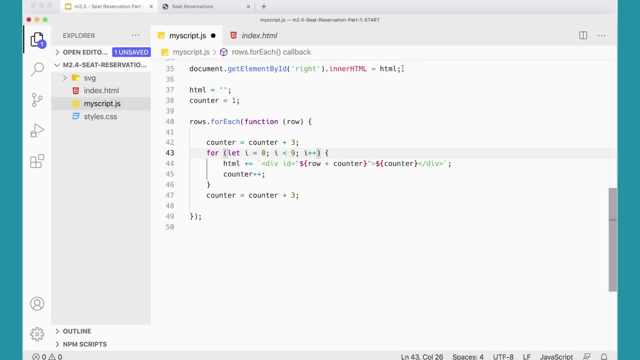 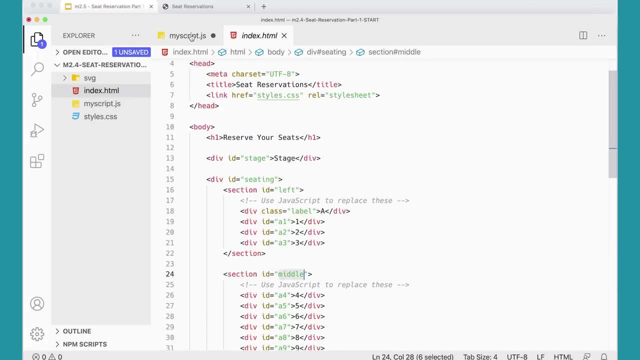 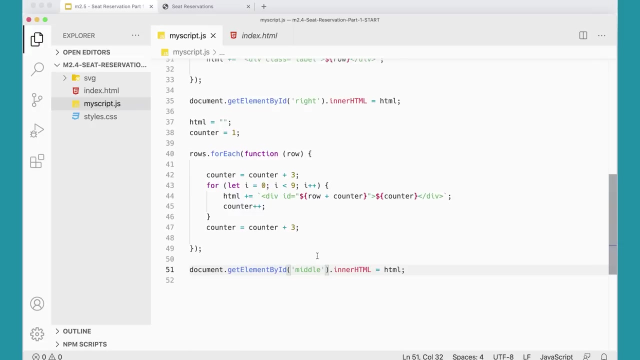 there, and then we just need to do this. but instead of setting it for the right side, we need to set it for- I called it center or I called it middle. we need to set it for the middle, like so, and that should work. let's go over and take a look. 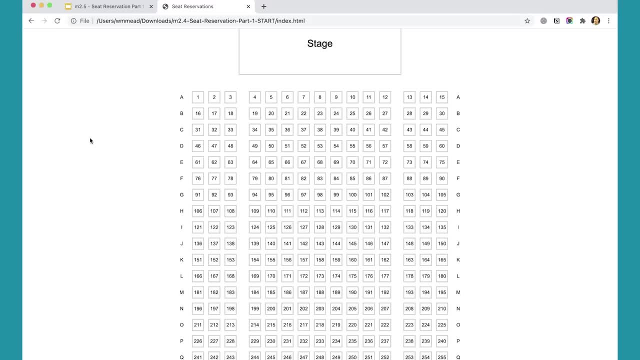 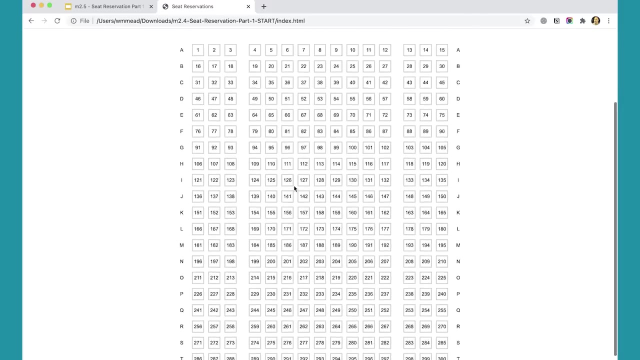 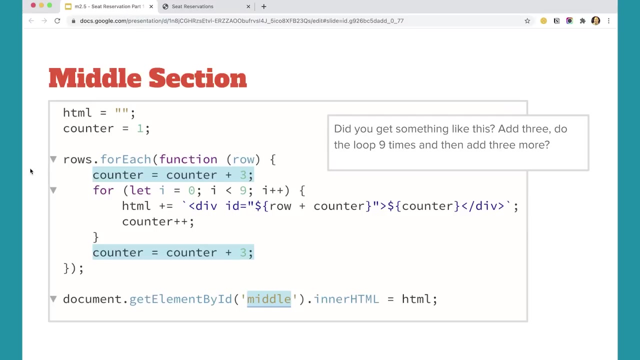 and look at that. so we have, at this point, essentially solved the problem I asked you to try to solve on your own, which is to create 300 seats, each with unique IDs and unique numbers. so we've done that and that's pretty cool and our script so far. 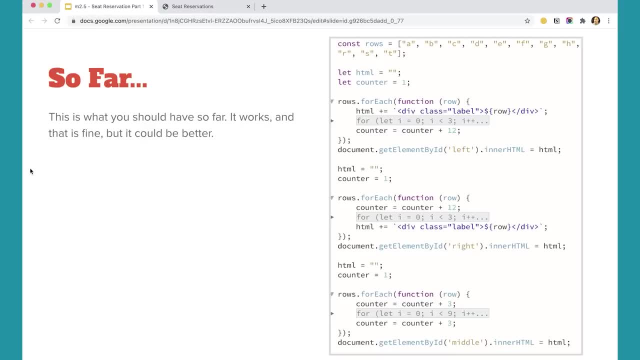 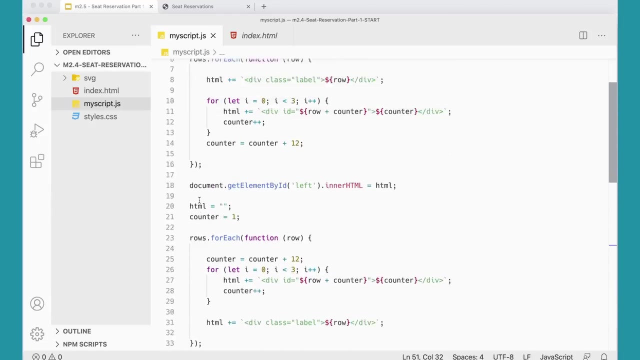 it's kind of long, it's kind of repetitive, so it could be better here. I have it shown over here in this image, with parts of it collapsed, or you can look at it here and kind of scroll through it. so we've got 51 lines of script here. 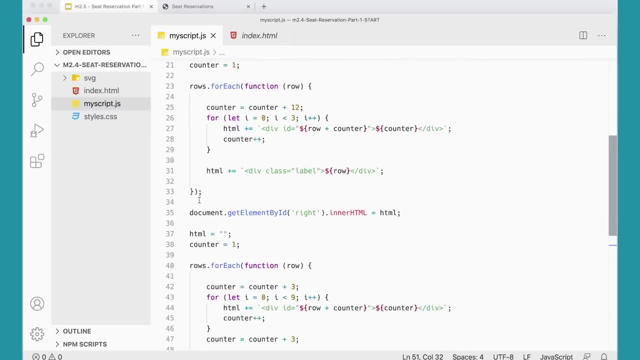 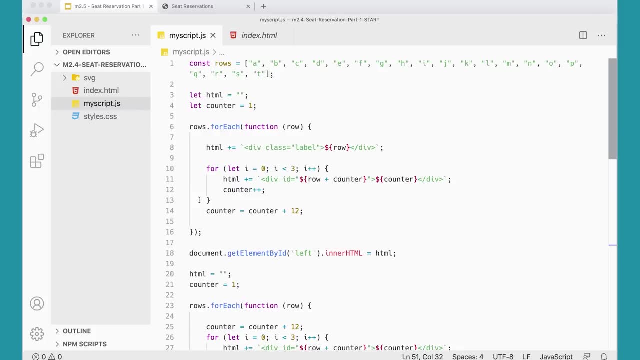 to create this stuff, but you'll notice a lot of the different sections are really doing pretty much the same thing, and one of our general guidelines is to not repeat yourself. so we want to refactor this down and make it a little bit better, I think, but we have essentially solved the problem. 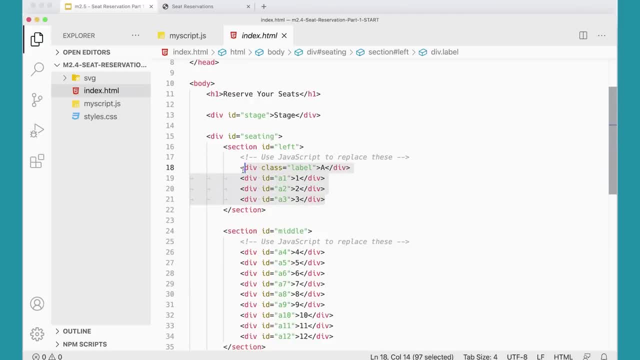 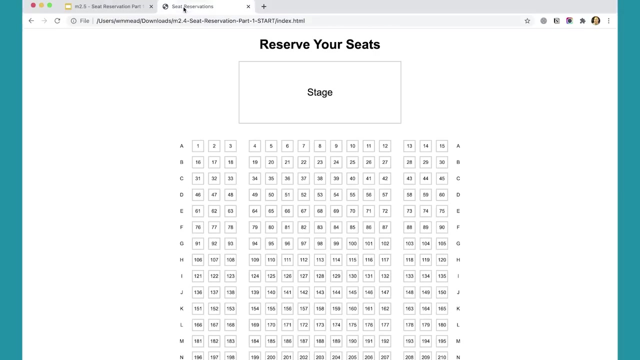 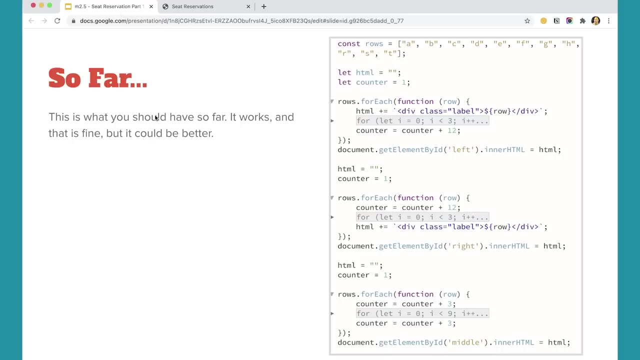 in fact, I can come back here and remove these built-in seats. we don't need them at all anymore so that our sections can be nice and clean, our HTML can be nice and clean and everything will get generated with JavaScript. because we were using inner HTML. JavaScript was removing that stuff anyway. 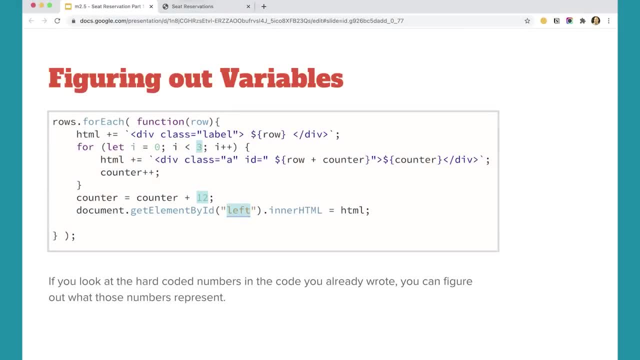 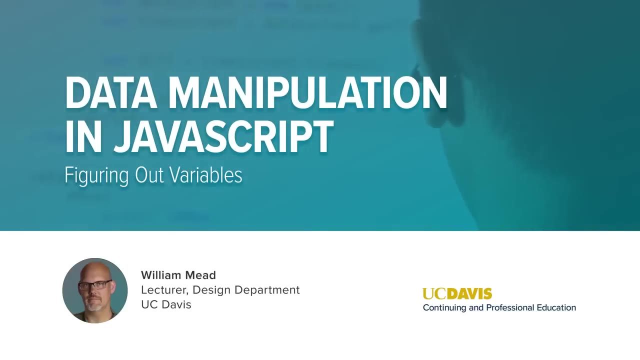 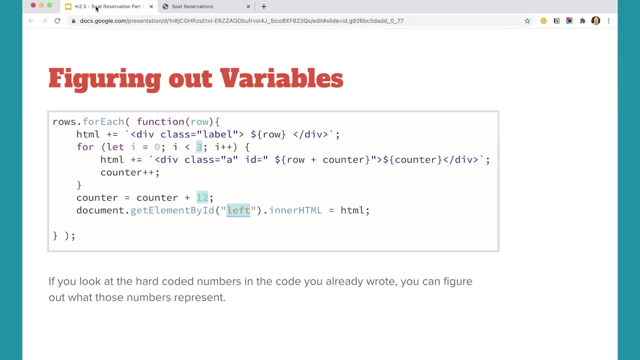 next we're going to figure out some variables, and we'll do this in the next video. we'll figure out some variables that we can use to help generalize our script a little bit more. finding out the variables: what we want to do next is take a look at the code we have. 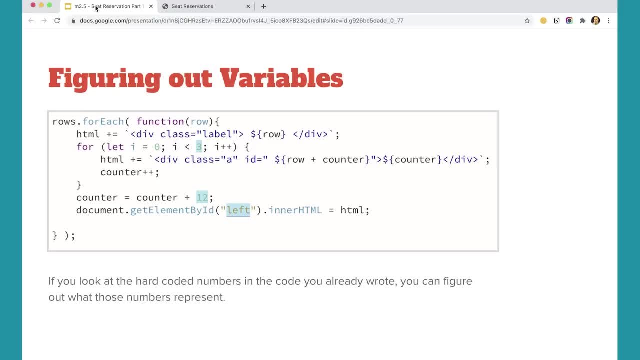 and see where we've hard coded some things in and see if we can find some ways of generalizing it. the idea is to create a function that we could use to create either the left section, the right section or the middle section- whichever section we need to- and that the function 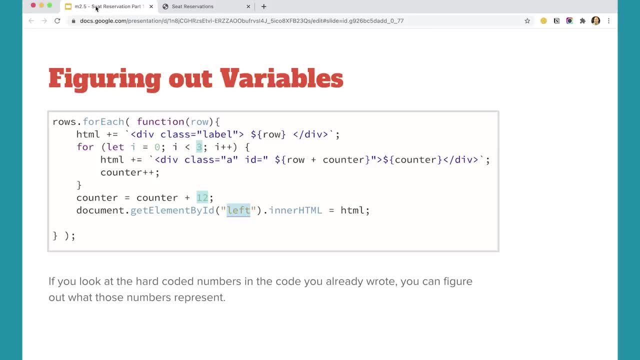 could be reused to do all three of those sections and handle the creating of the seats for each section as we need to. so as I look at this, I see: okay, we've got a 3 here and we've got a 12 there, we've got the place. 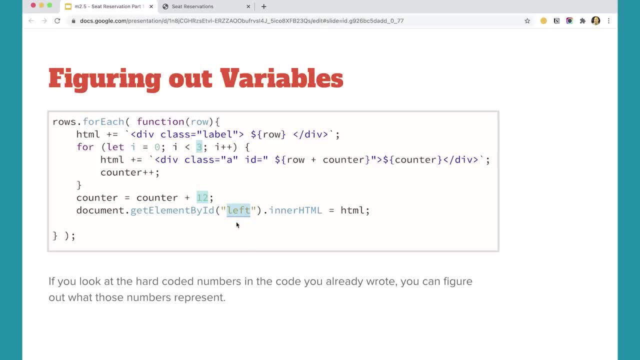 where we want to put it and what I figured out is. I need to know 3 things. I need to know how many seats are in the section for the row that I'm working on. is it 3 or is it 9? I need to know how long. 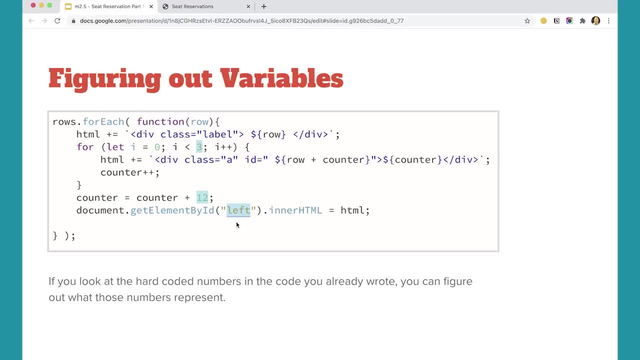 that total row is so in this case it's 15, and I also need to know which section am I currently placing seats in. am I placing it into the left section or the right section? and those are the things that I need to know: the left section, the right section. 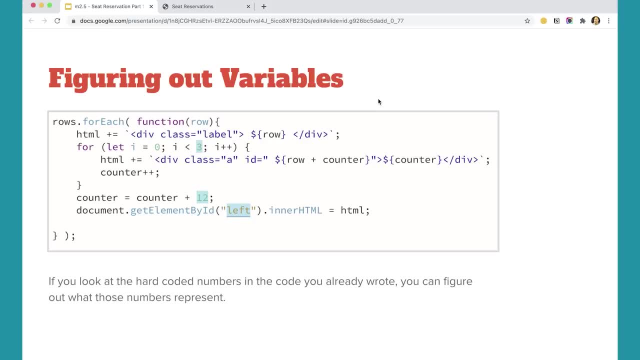 or the middle section, any of those sections. those are the 3 things that I need to know: how many seats am I putting in, how many seats total are there in the row and which section am I working on? so this is where we are going with this. 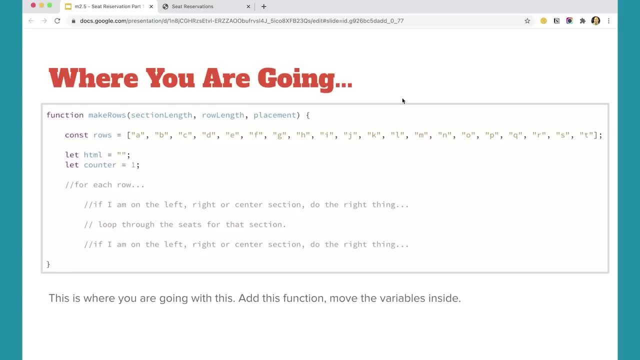 we're going to make. we're going to have a function that makes some rows and we're going to create those 3 variables- section length, row length and placement- and we can put our variable for our rows right inside there in our initial HTML and counter in there. 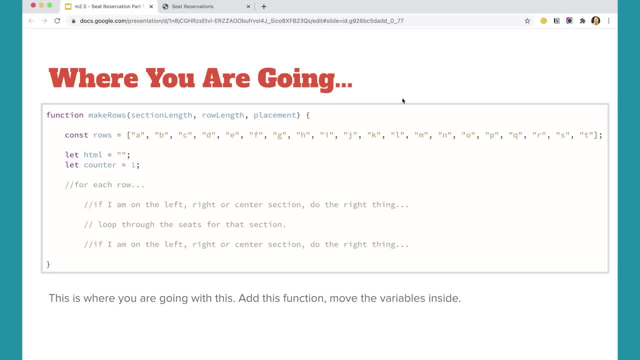 and then, if I'm on the left or if I'm on the right section or in the center section, I need to do the right thing. I need to either put in a label if I'm on the left or not, or not put in a label if I'm on the right. 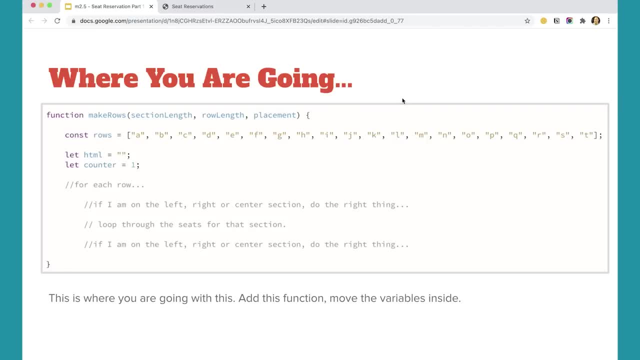 you know, however it is, I need to do the right thing there, and then I need to loop through the seats and then if I'm on the left, I'm done, but if I'm on the right I need to have the label, and if I'm in the middle I'm done. 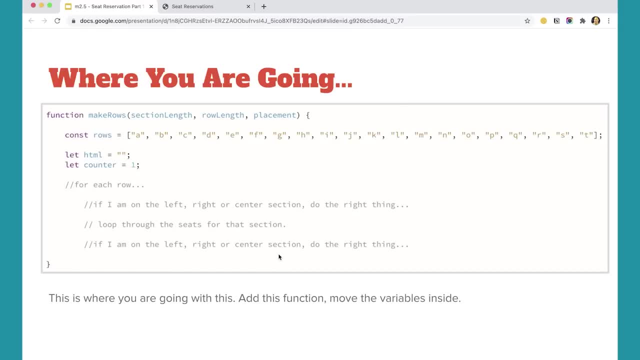 so I just need to have this kind of structure going on. that's where I'm going, that's where we're going to go with this, with my solution anyway, and perhaps you came up with something different, and that's fine, so let's try to see if we can figure out. 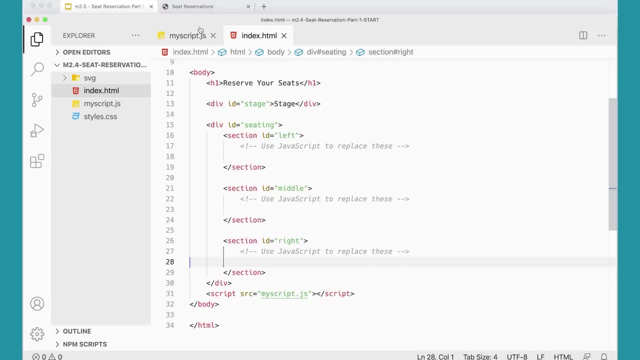 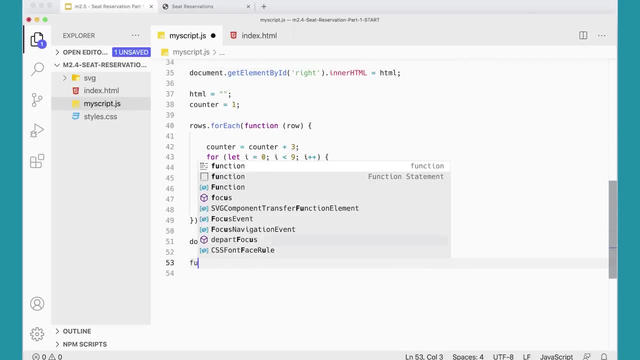 that over here on my script file, I'm going to make a function. I'm going to just put it down here for now. function: make rows and it needs three. it needs three parameters: section length, section length, row length, row length, row length and placement and placement. those are the three things. 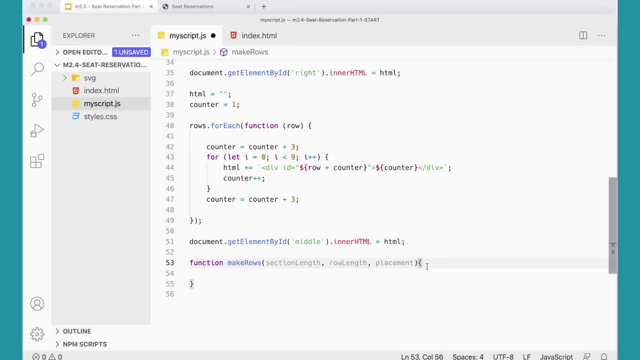 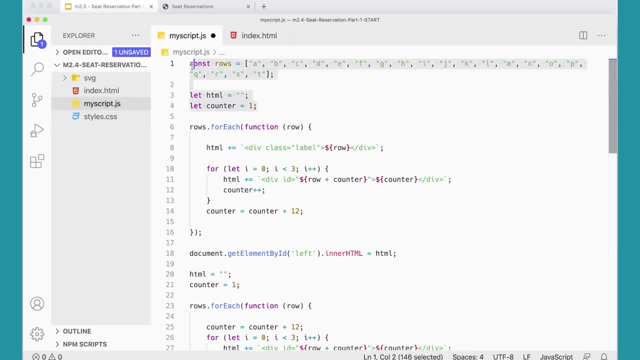 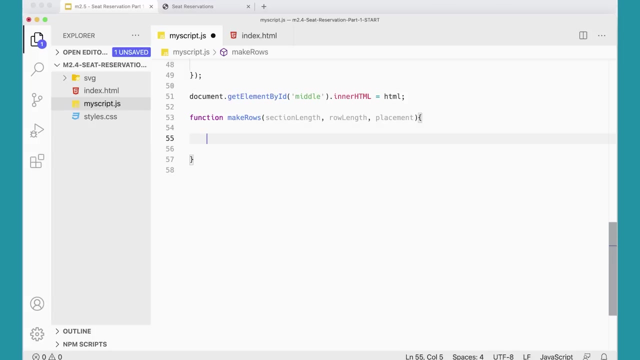 I need to know to make this function work properly, and then I can. I'm going to just copy and paste this stuff from here, because we'll comment all this stuff out or delete it later, but we can get these going right inside of our function here, okay. 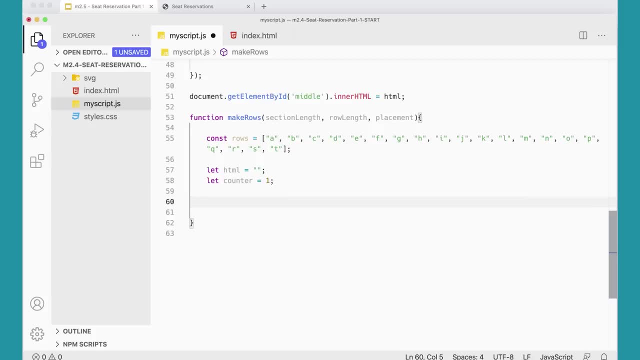 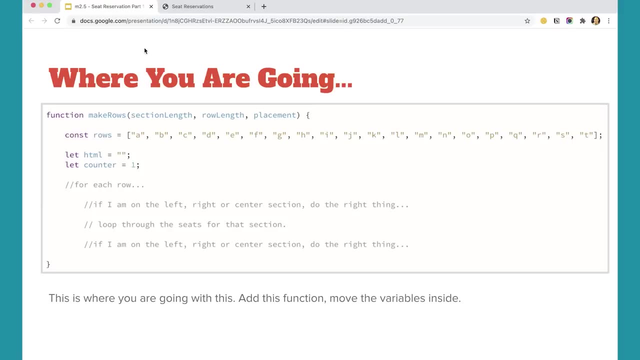 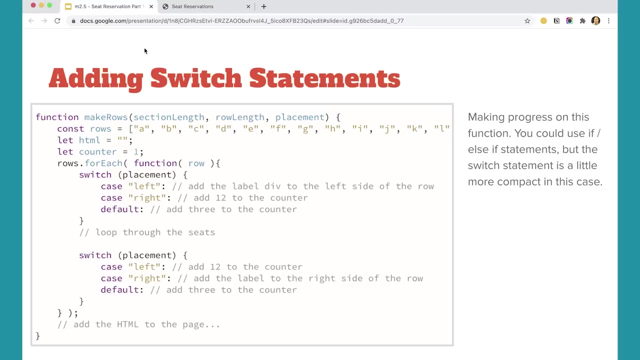 so we've gotten it started, and then we need to think about what we're going to do next, and in the next video we'll add these switch statements that will hand all what we're going to do if we're on the left, the right or in the middle. 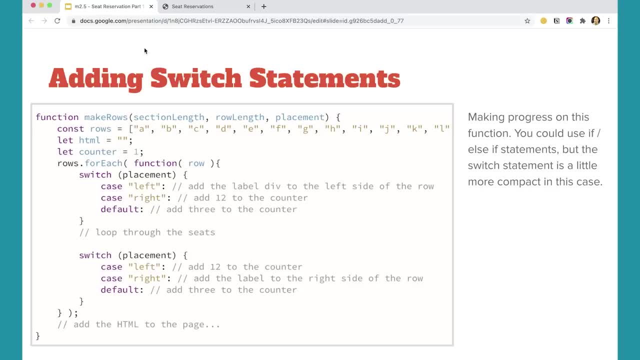 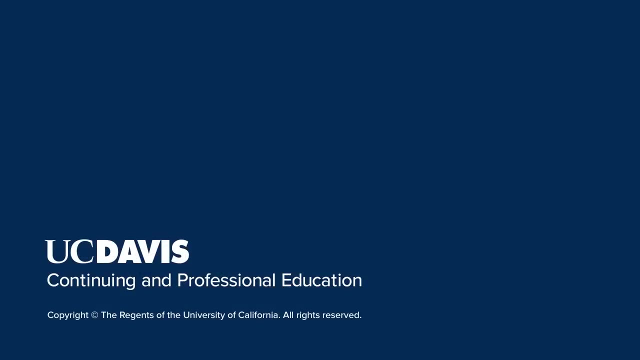 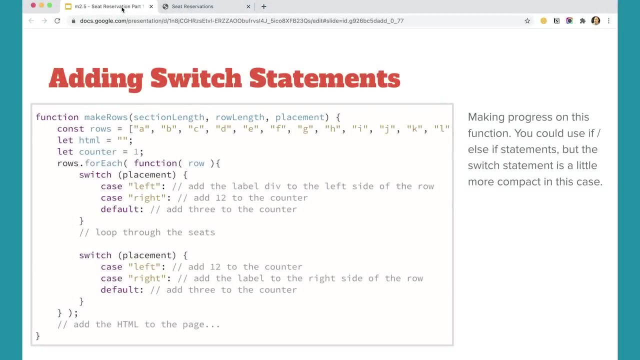 and I'm going to use the switch statement just because it's a little bit shorter than shorter syntax, than if else statements, but you could use if else statements. but we'll see what we need to do with that. we'll use the switch statement to determine what we need to do for each. 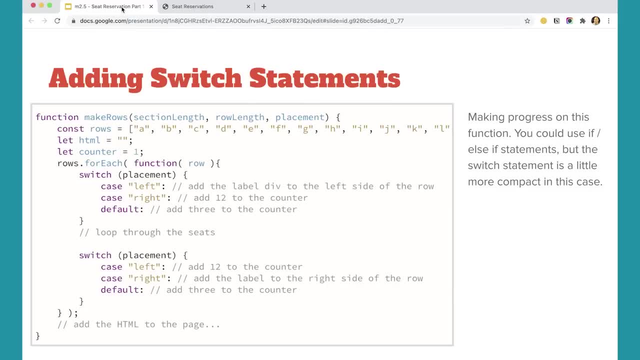 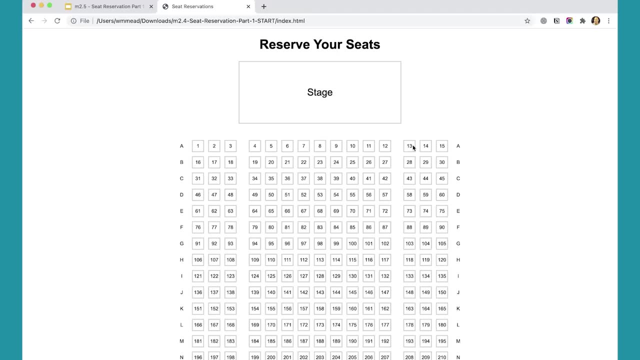 for each section, depending on which section we're currently filling out. so if we're working on this section, we need a label and then three seats. if we're working on this section, we need three seats, then a label. if we're working on the middle section, we just need to skip. 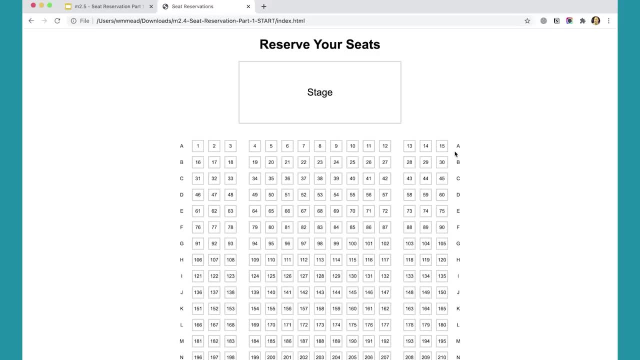 three seats, work on the middle section and then skip three seats. we don't need a label at all. so depending on which section we're working on, we're going to do different things up front. so let's get started with this. the first thing we're going to do is: 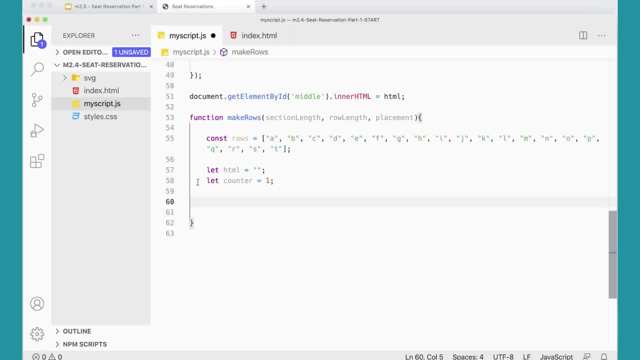 we're going to need is our for each loop. so we'll take rows and add our for each loop and we could copy and paste from above. but I'm going to just type it here: function, parentheses, curly braces, semicolon, and in here I press return and I'm going to make. 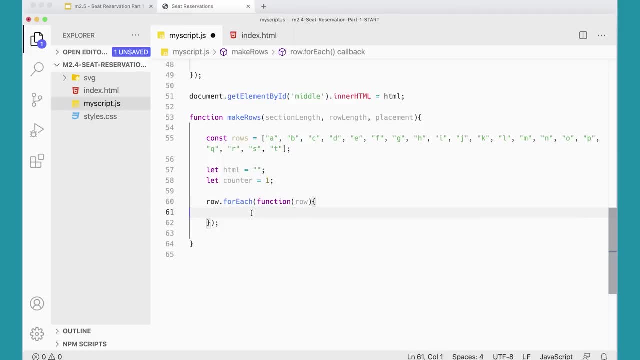 rows. so there's our for each loop and then, based on which placement is passed in here- left, center or right- which section are we working on? so I'm going to do switch placement like this and in here we're going to have a case, the case for. 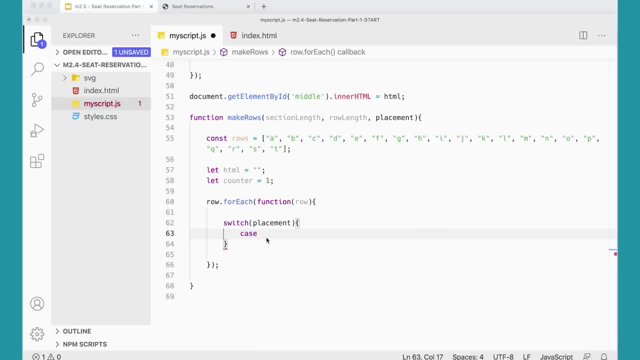 for left, if we're working on left. if we're working on left, we need to make the label label label, label, label case. if we're working on the right, oops case, right, right. if we're working on the right, we need to add 12 to the counter. 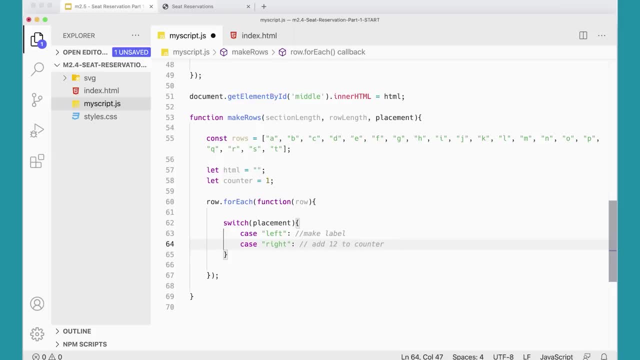 12 to the counter, basically right. and then if we're not working on the left or right, then we can say: well, the default is we're on the center default. yeah, there we go. and if we're working on the default, then we're going to add: 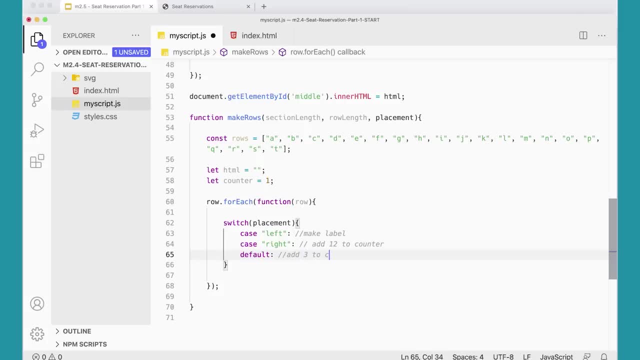 three to the counter to begin with. so that's one switch statement and we could do this with else ifs. but I think the switch statement is a little bit more compact after we've either created the label or added the right number of seats to the counter. right number of. 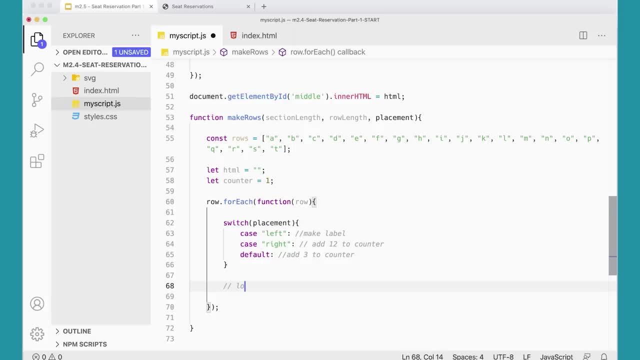 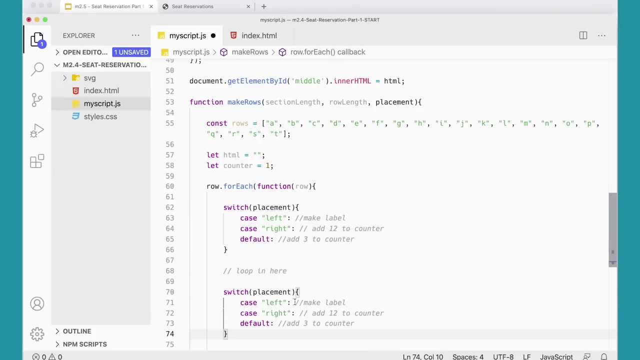 numbers to the counter, then we're going to add our loop, so our loop will go in here to make the actual seats. but then we need to do the right thing on the other side and we can just copy that and paste it. and if we're on the left, 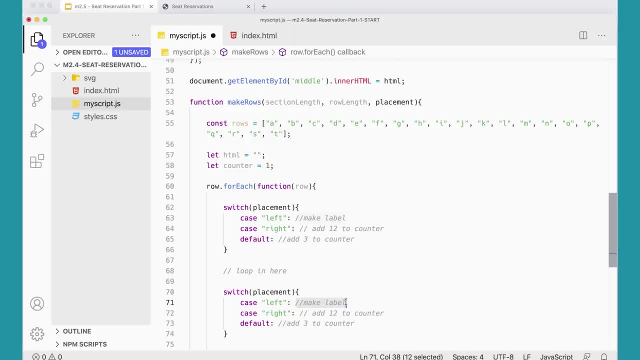 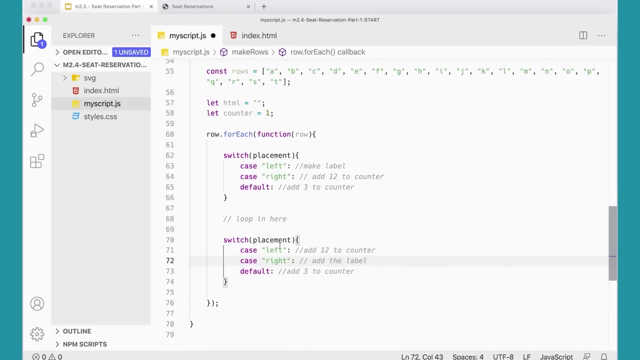 this is where we're going to add, add, add 12 to the counter here, whereas if we're on the right, that's when we're going to add the label and the center section is going to add three to the counter either way. so that gets sort of a basic structure. 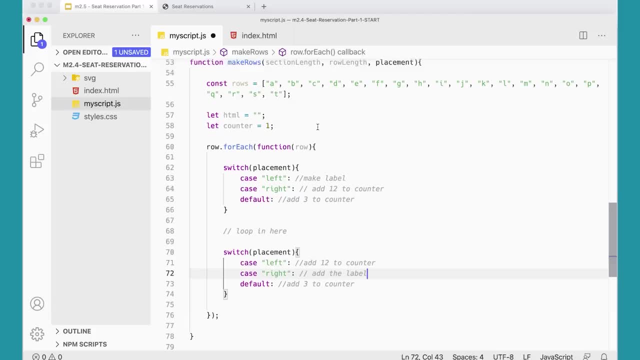 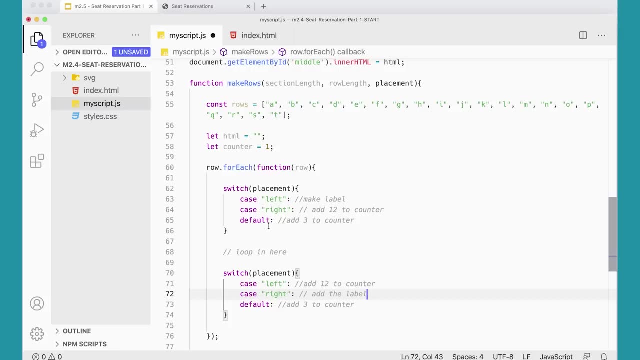 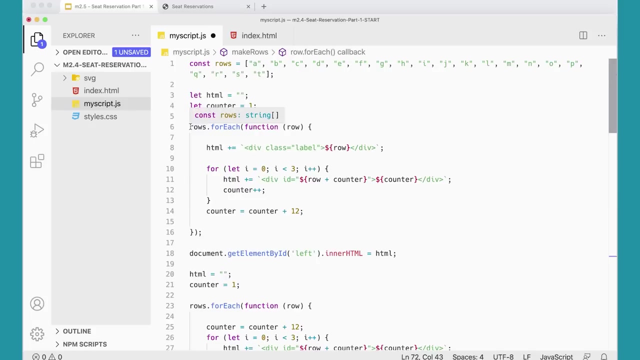 for what we're going to do, based on which side we're passing in to this placement variable. here we're either going to, we're going to do something here and again. what we're doing is sort of refactoring this stuff down and seeing what the difference is. 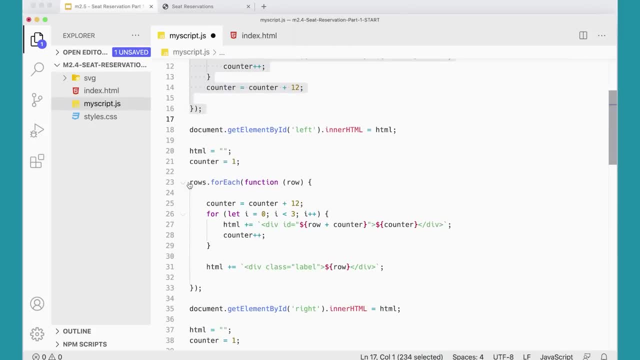 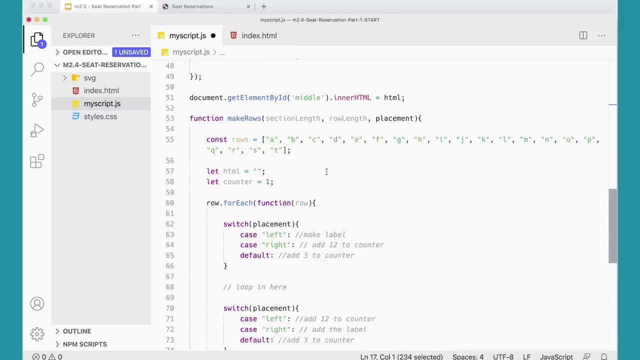 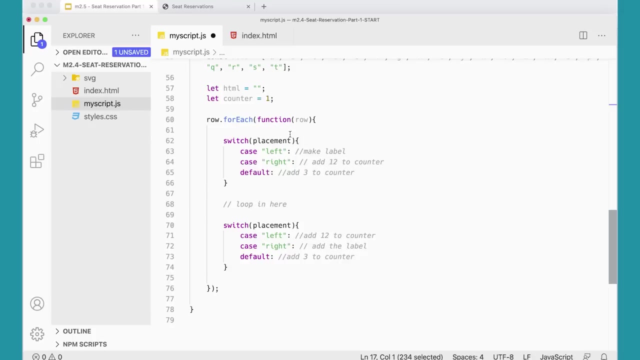 well, what's the difference between this one and this one? and the difference here is that we put the label first and then add the counter to 12 at the end, so you can see that sort of taking place down here. lets go ahead and fill out these. 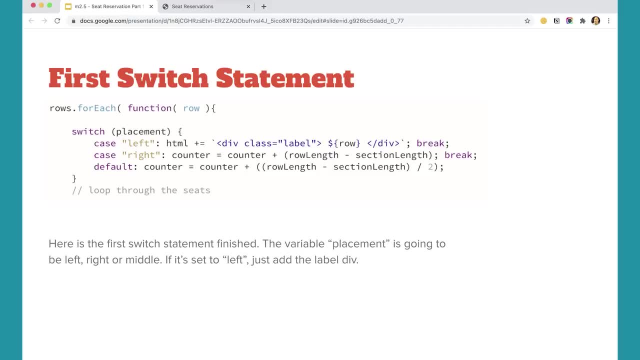 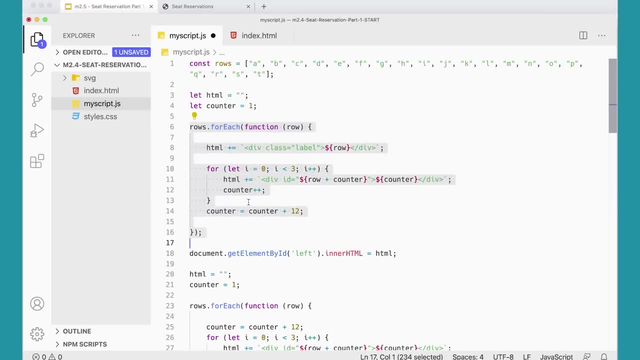 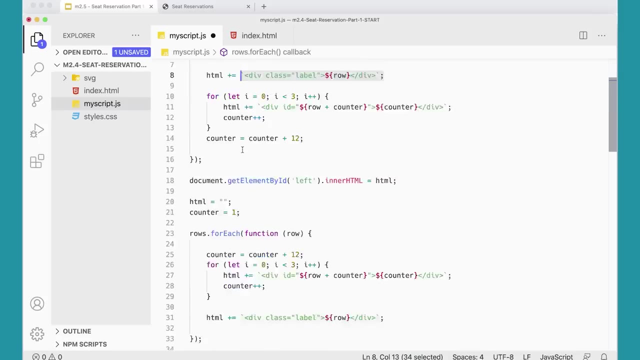 switch statements. so for the left one, it's pretty straight forward. we can actually go up here and steal from up here. so we're basically just going to do this. you can type it again if you wanted to, but that's what we're going to do here. 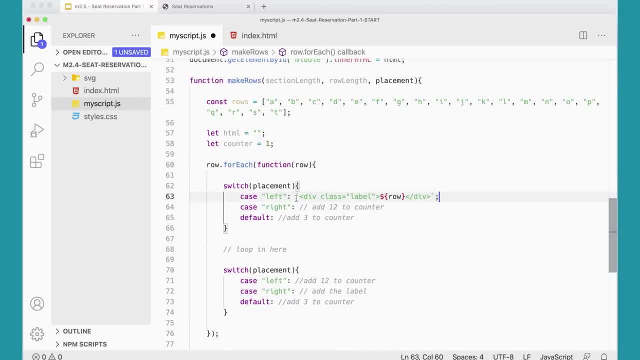 we're going to make the label which is setting the html equal to that, that div. so we're going to set that, set that variable html. I'm going to do plus equals, plus equals, that thing there. and then at the end, don't forget to add break. 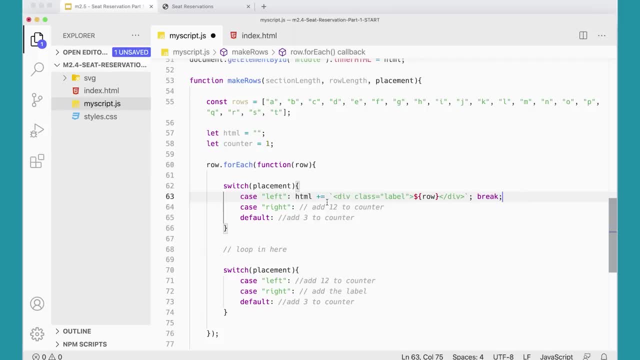 when you're using a switch statement. if this one is true, you need break to break out of the switch statement there so that it doesn't try to go on and do the next thing. so if you forget break, then the switch statement will not work properly and you'll be chasing around that error for a little while. 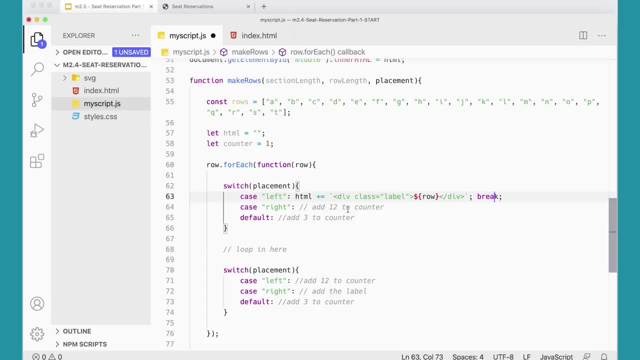 so we've got that in there for the right side. what we really want to do is we want to say: well, counter is going to be equal to- I'm going to use parentheses here- the section: the row length minus the section length: row length minus section length. 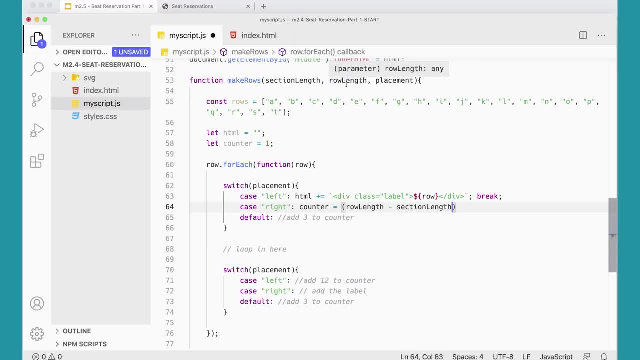 because the row length is 15 and we're going to subtract the section length, which is 3, so that's going to give us our 12 right there. so that's what we need right there and then down here what we need to do, for the default is we need to get. 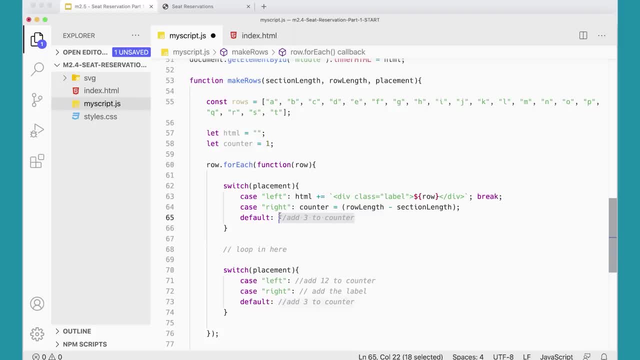 3. so it's really, if we're in the center, then the section length is 9 and we can subtract that from the 15 and we'll get 6 right. so we need to take that and divide it by 2. so down here we're going to say: 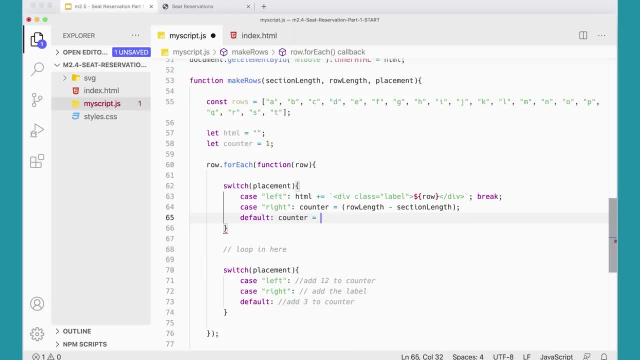 counter equals the row length minus minus the section length right. I'm going to put parentheses around that divided by 2, and that will give us 3 on that side. on my image, I had an extra set of parentheses around the line, so I'm going to. 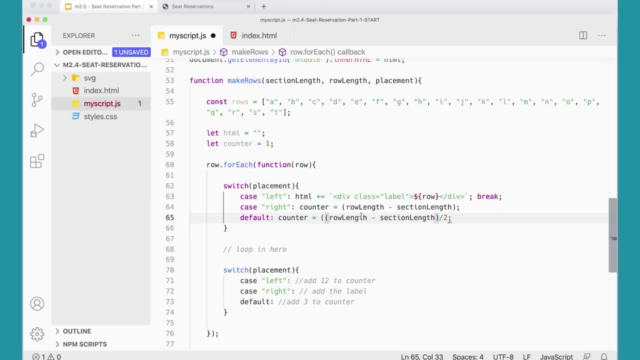 I'm going to. I'm going to do the whole thing just to make sure it all works properly. it probably doesn't really need it, but the counter is going to be the row length minus the section length. I want to do that first. I want to take that row length. 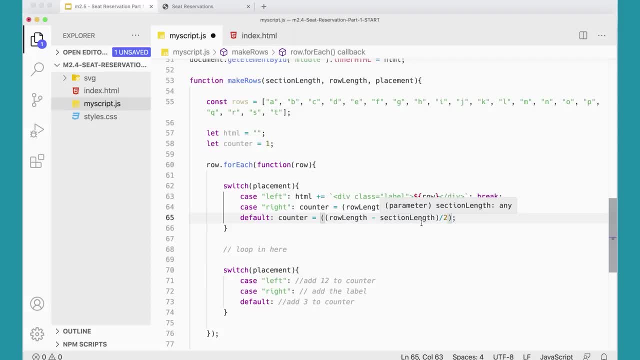 which is 15 minus the section length, which for the center is going to be 9, that gives me 6. divide that by 2 to get 3. so that's great, so that works. and then down here it's really just the opposite. well, this one's the same. 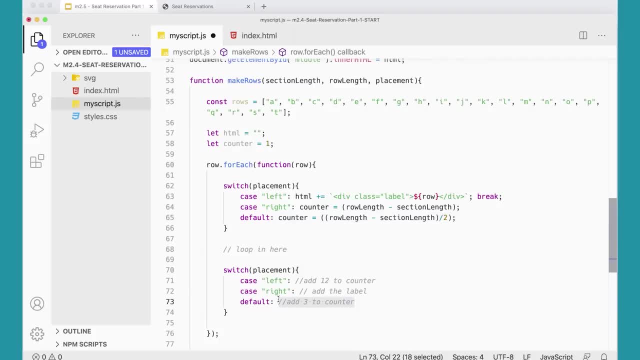 so we can copy this one and stick it down to the bottom, but left this one here. in case of left, that's actually going to be what goes on the right hand side. we're going to make that label there, and right is going to get the counter setting. 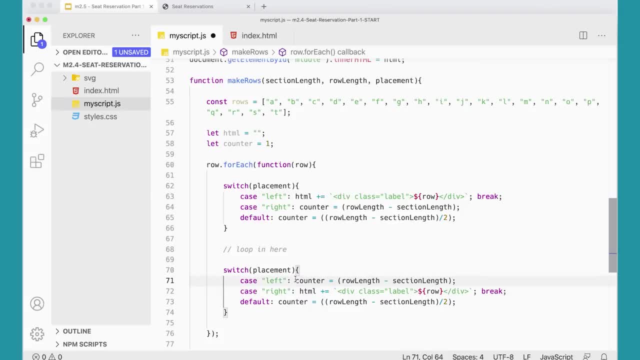 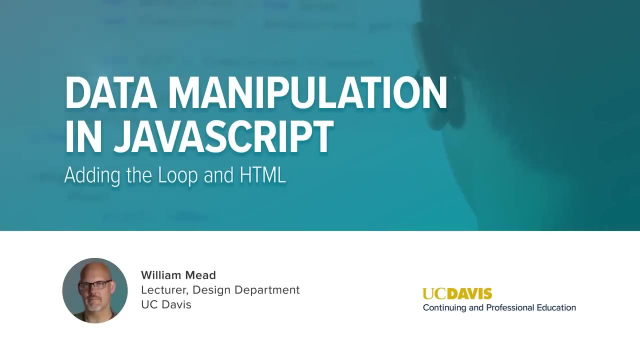 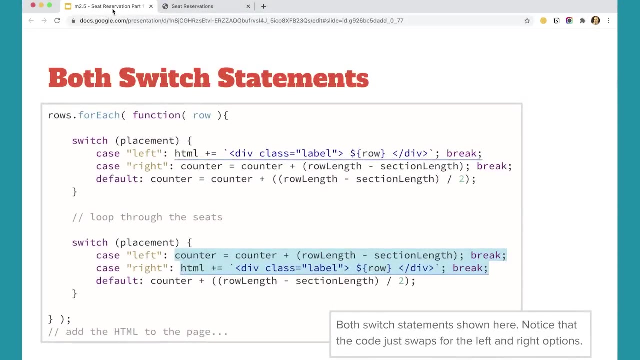 I mean the left is going to get the counter setting there. so that kind of sets our switch statements up and then next we just need to do the loop and we will have this function pretty much done. we've added the two switch statements to our function so that it will handle. 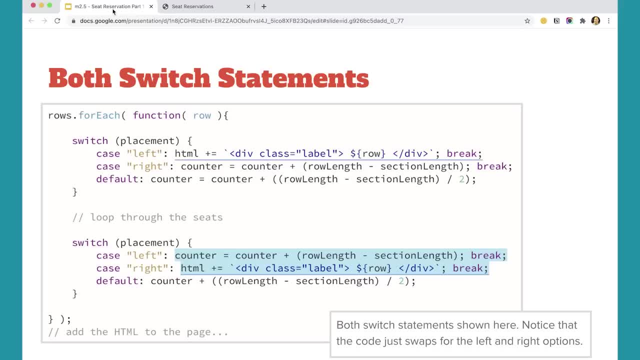 the correct HTML on either side and the placement, the correct numbering for the, for the different boxes and the different sections, the different seats and different sections. now we really just need to add the loop and again the switch statement down here. they're just kind of swapped around because that's what's going on. 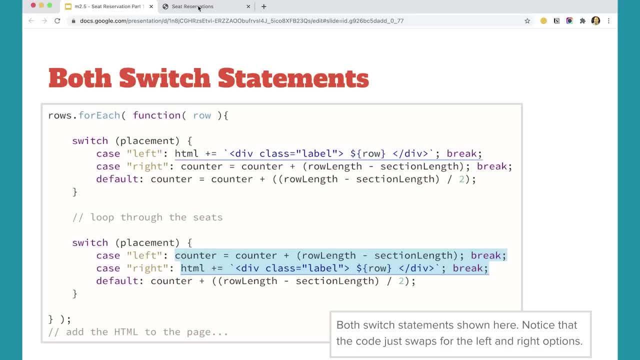 with what's going on over here, where on the left we have the label, over here we have the label on the right, so they're just sort of swapped around in order to get that effect, okay. so let's take a look at the loop, and the loop is: 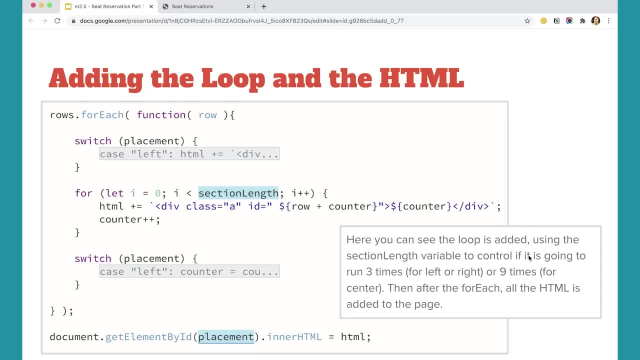 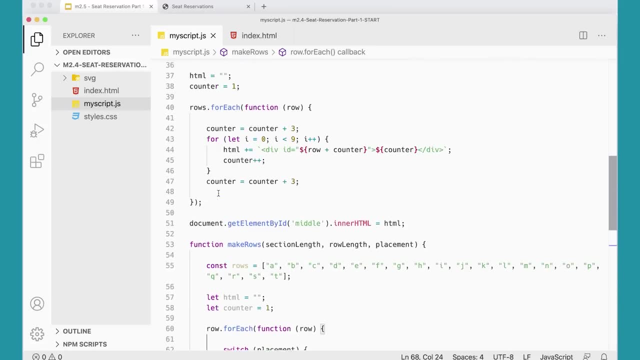 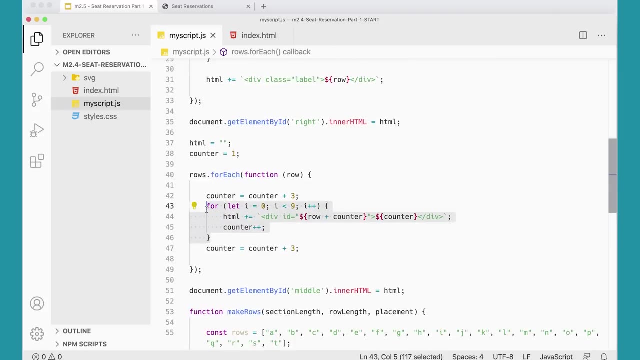 fairly simple, in fact. we can just copy and paste the loop that we have from up above and just make some minor changes. so up here it's really just this same loop, right here. I can just copy this one and stick it in where it says: the loop goes here: 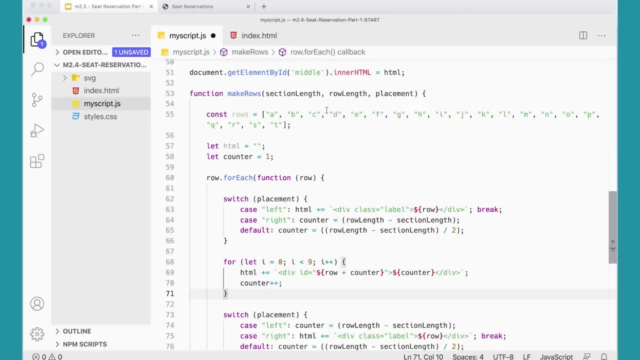 but instead of nine, what we want is the section length. we want that variable because this loop is going to be used for the seats on the left side, for which there are three. it's going to be used for the seats in the middle, for which there are nine, and the seats on the right. 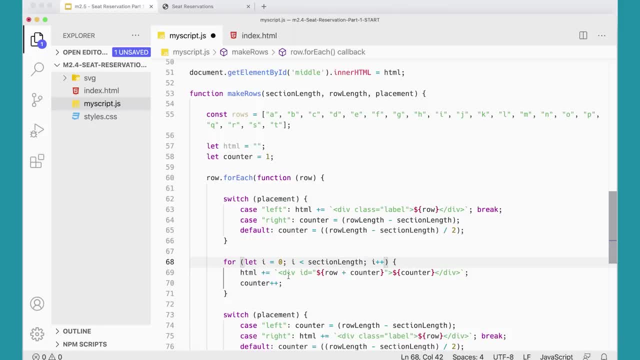 for which there are three. so we want to do that. one other thing that we want to do is we want to add a class in here. class equals quote a, and this is going to become important later when we determine whether seats are available or not, so don't forget that. 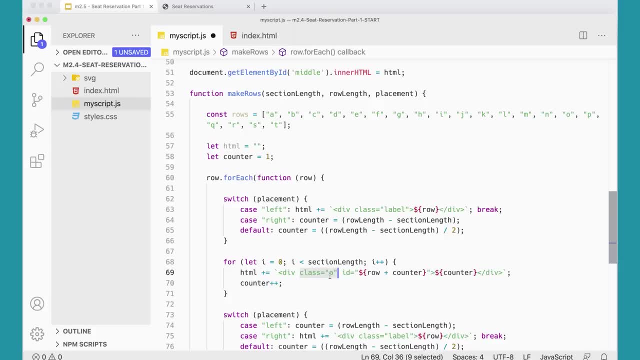 to put in this class equals a here, because a is going to stand for available. so these seats are all available and as they get reserved we'll change that class to an r and as you're clicking on seats in the little web application there, they'll get changed to an. 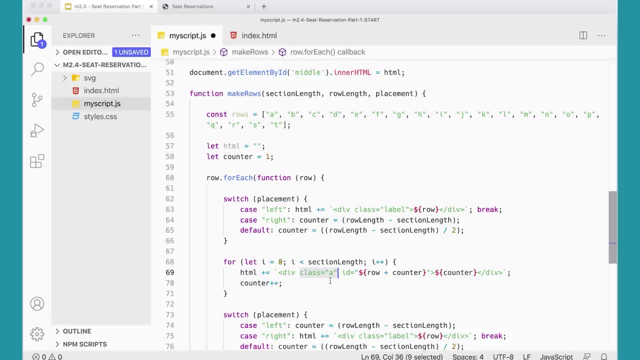 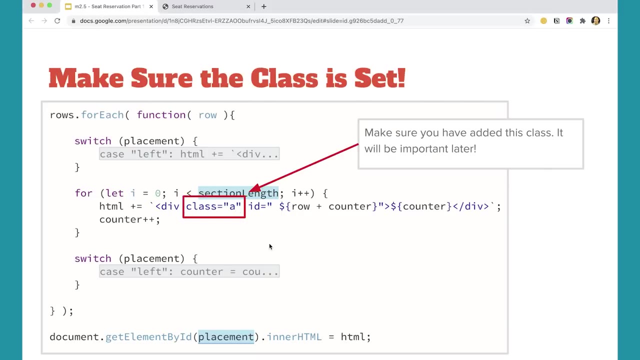 s for saved so we can hold, keep track of which seats are doing what and what their state is currently. so we need class equals a on there and again, just to reinforce that, i have that here as well: class equals a. make sure you add that, because otherwise it'll get screwed up. 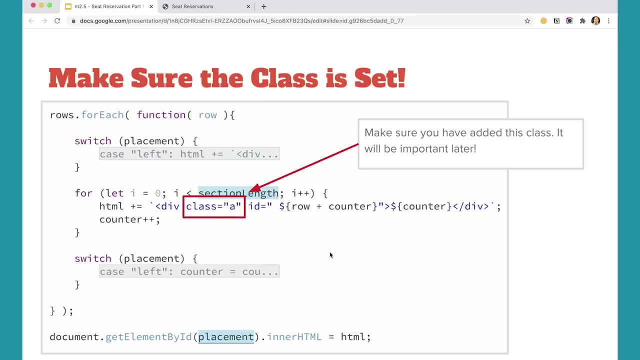 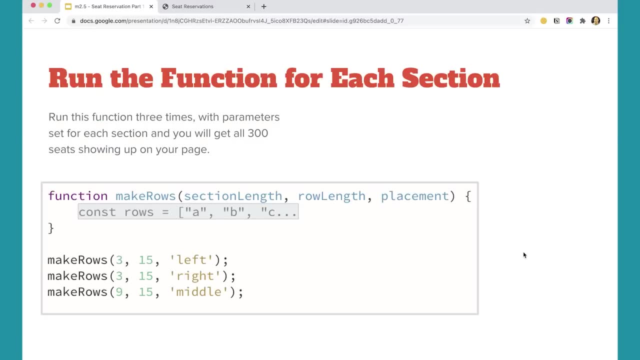 later. okay, great, so we've got our loop in there. we're ready to give this thing a try. what we all we need now is to call this function three times, make rows 315 and left for the left side, 315 and right for the middle side, and. 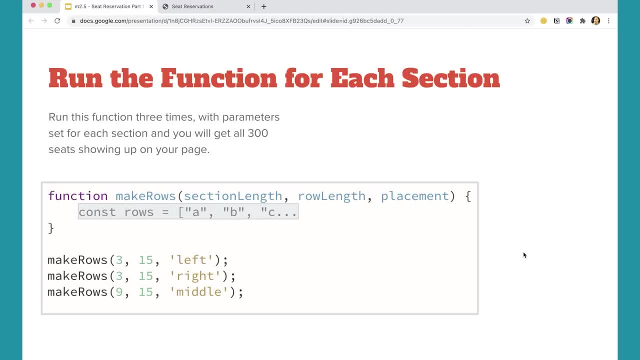 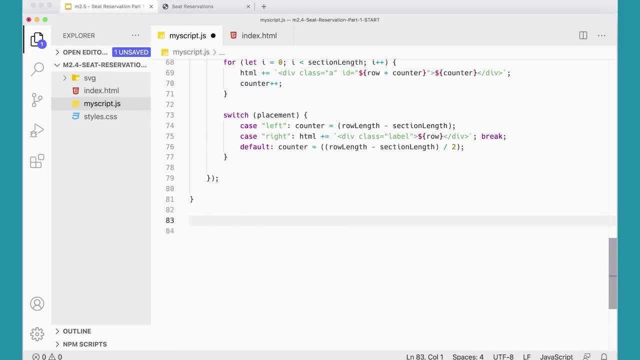 915 for the middle side. sorry, 315 right for the right side and 915 in the middle for the for the middle. okay, so let's do this and give it a try. so down here i'm going to run, make rows 3, 15 and left. 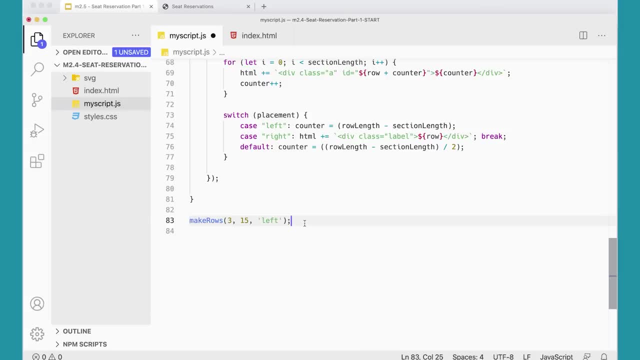 that's the left side and you could do the right. i'm going to record that last bit again because the dog was barking. all right, let's start here. we're going to call this three times, make rows, and we're going to do three for the left side with 15. 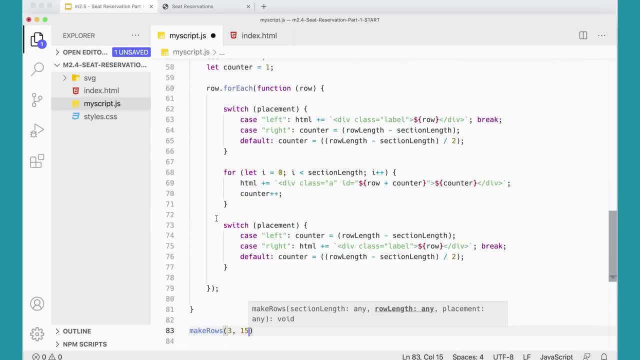 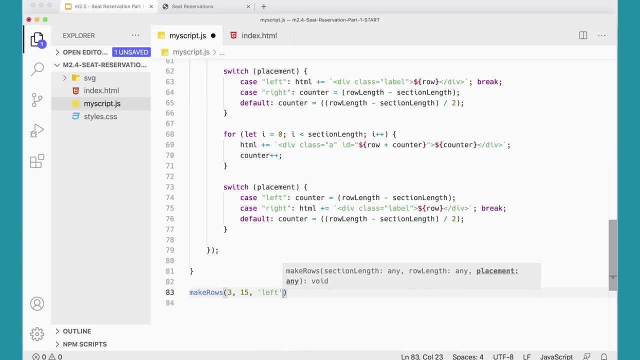 three is the, the section length, the rows. the row length is 15, and then we're going to put in left and that's what we need for the left side, and then then we'll do make rows again, but this one's going to be right, and then 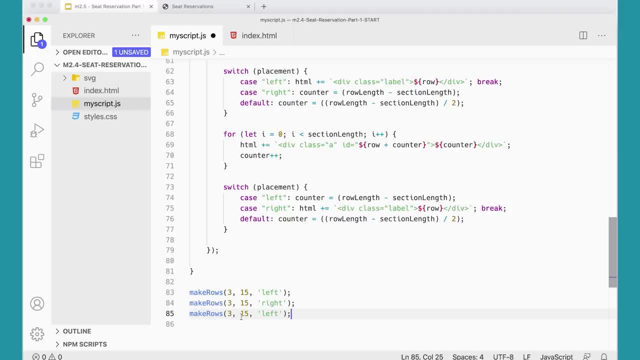 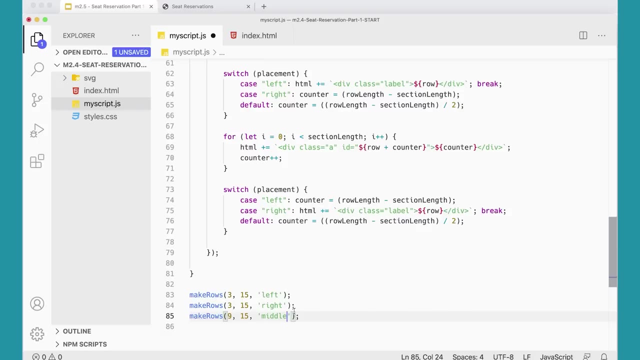 we can do the center. so that's going to be how long is that one? that's going to be nine and that's going to be middle. so we, we're running, make rows three times to create, create this, create all the seats here and then we can come up here. 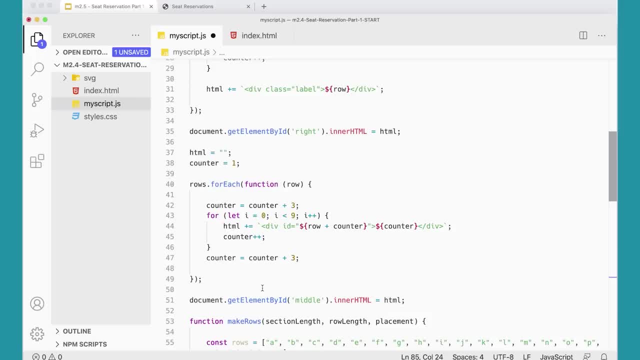 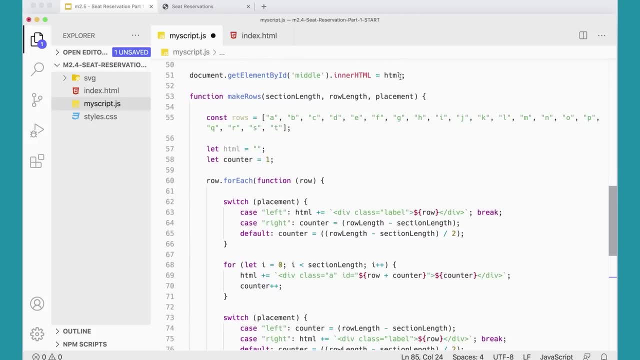 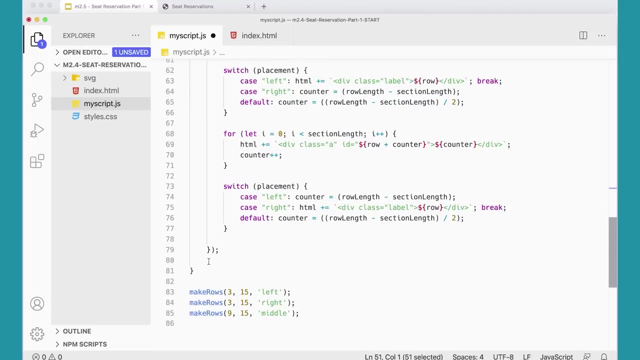 and get rid of all of this stuff i did. i'm realizing i forgot one thing in make rows here. i forgot to add this: you need to actually put the html on the page. so down here in make rows, we're going to come in and do placement. 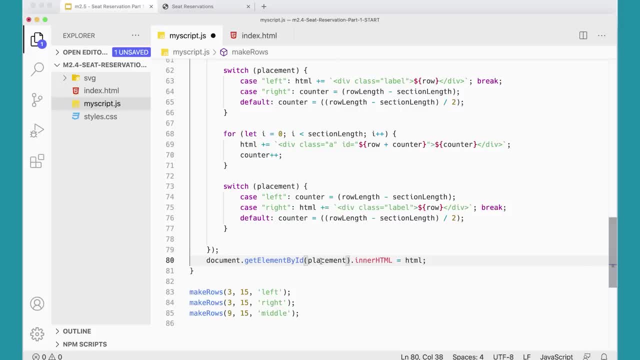 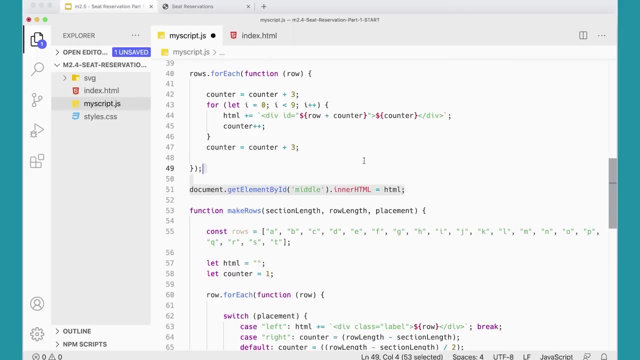 and get element by id placement, so it's either left, center or right, or left, middle or center or whatever it is there, and we'll put that in our html in there. forget to put that in there, so that's going to be important, but up here we can get rid of all the. 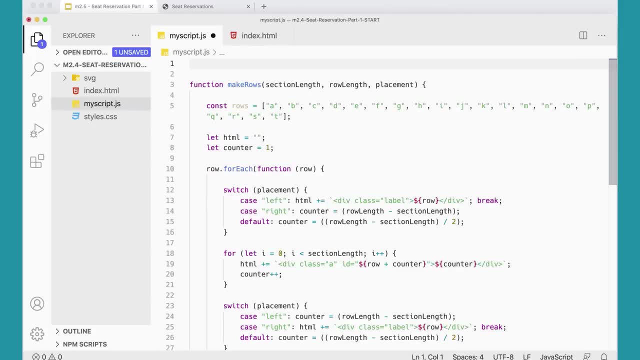 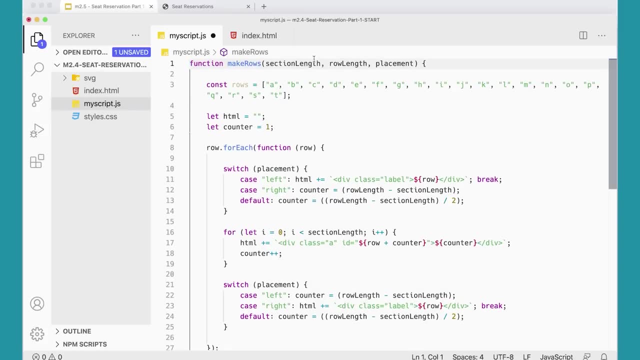 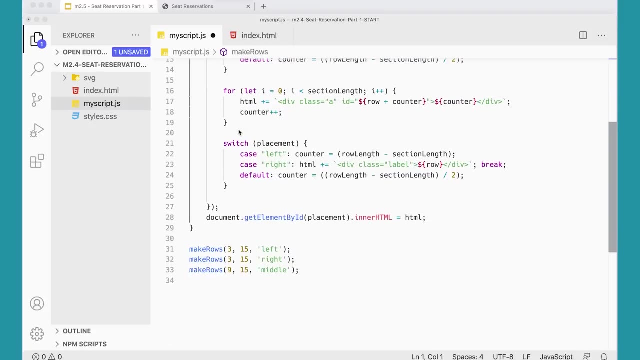 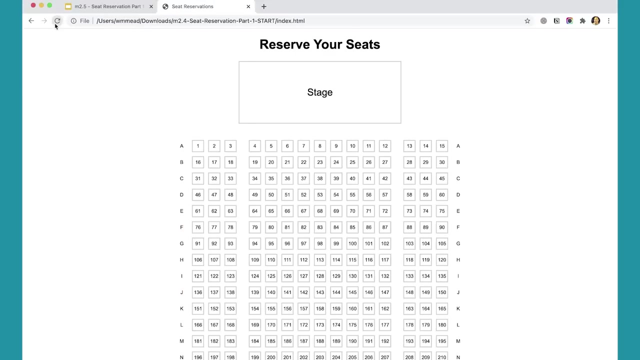 rest of this stuff all the way up to the very top. so we just have a function called make rows, make rows with our variables in there, and then calling make rows three times. let's see if this works. oops, i must have a error in here somewhere. 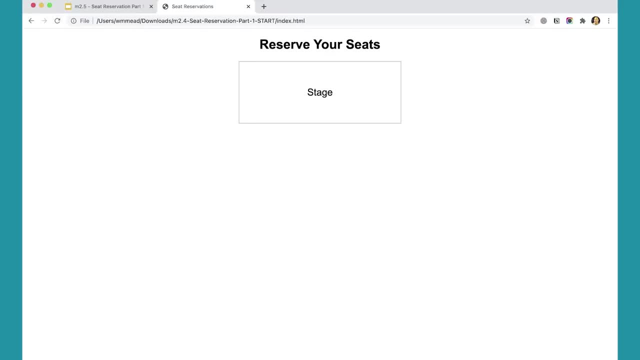 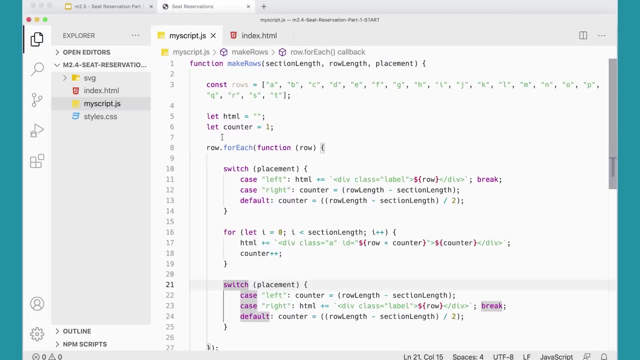 let's go and inspect and, sure enough, i have an error here. console row is not in here, and so i'm going to call defined on line eight. what did i do wrong over here? rows- that needs to be rows. there we go and, whoops, something went wrong. 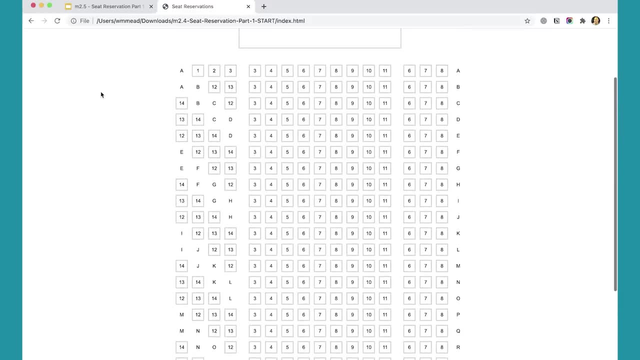 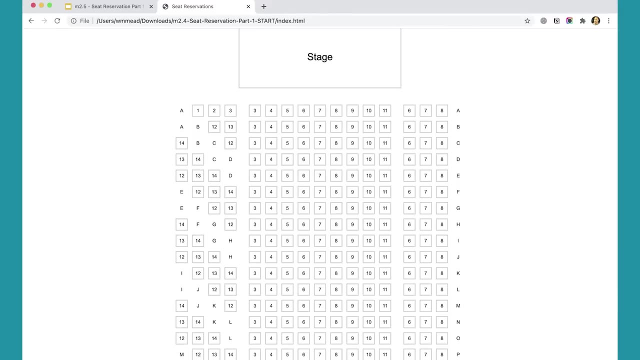 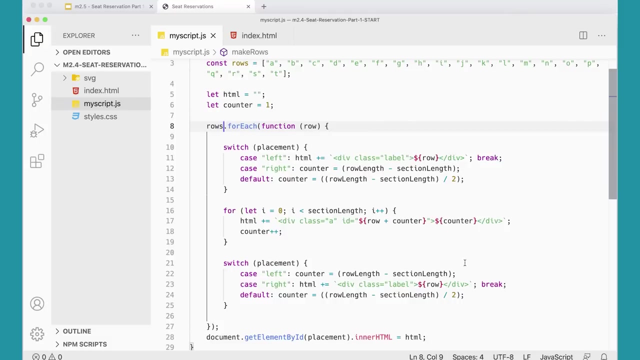 on my left side. let's go take a look and see what. what happened with that? remember i mentioned you have to put the break in. you can see i forgot that. so i need a break here and i need a break here down here. i need a break here. 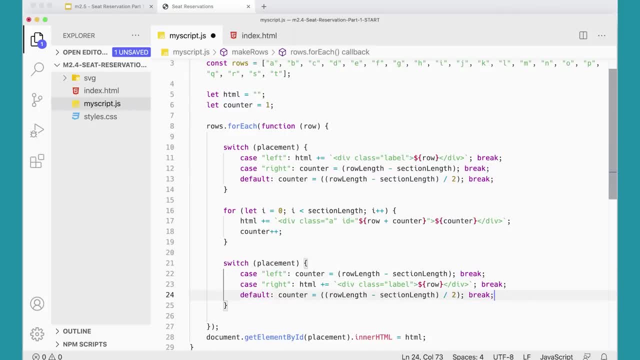 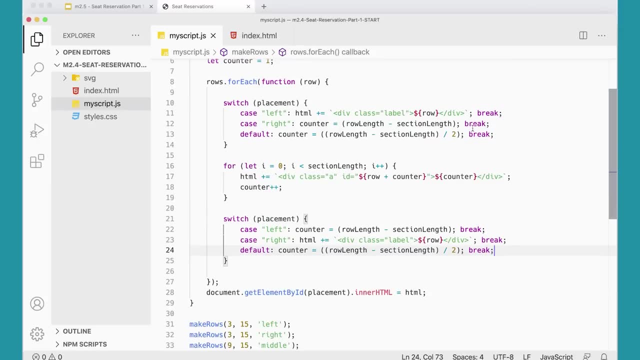 and a break here down here. i had made a big deal of that in the video because i often forget to add the break in the switch statements, and then i did. so these kinds of things happen, so you just have to go and see what's going on and see if you can figure out. 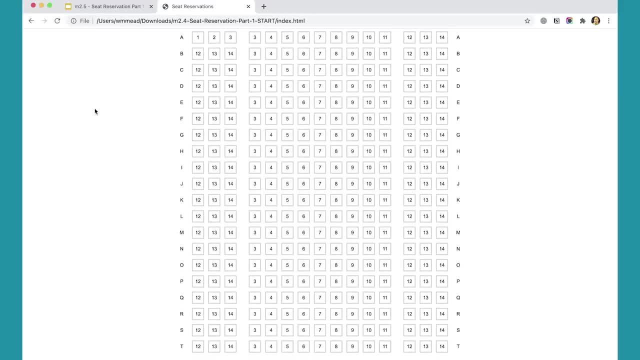 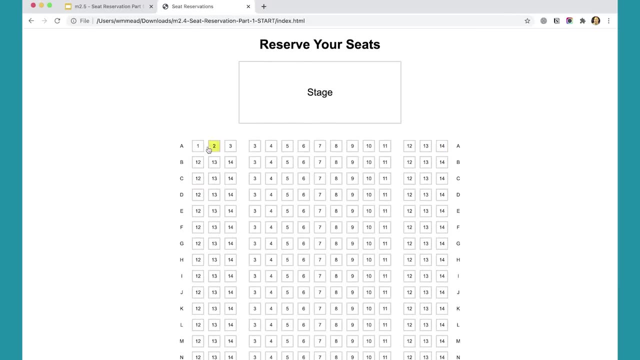 what the heck is going on there. and look at that now. it's perfect. well, not perfect, it didn't do the number incorrectly. it didn't do the number incorrectly. the right side, the right side- 12, 13, 14. we're getting three there, so that's not right. 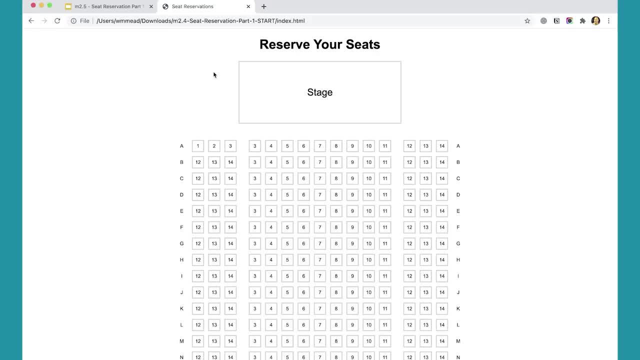 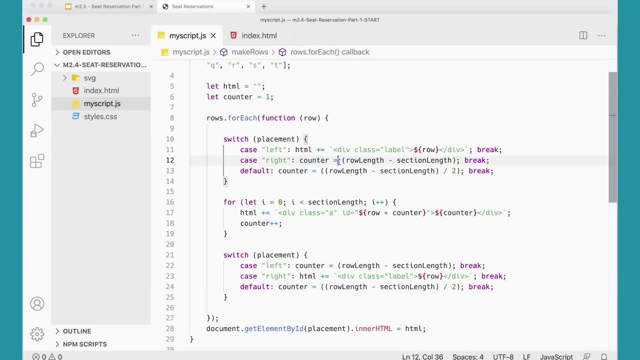 that should be four. that should be four. i see what i've done wrong here. i see what i've done wrong here. this needs to be counter equals counter plus row length, and then down here: counter equals counter plus, and then the same thing down here. okay, let's go back and try it one more. 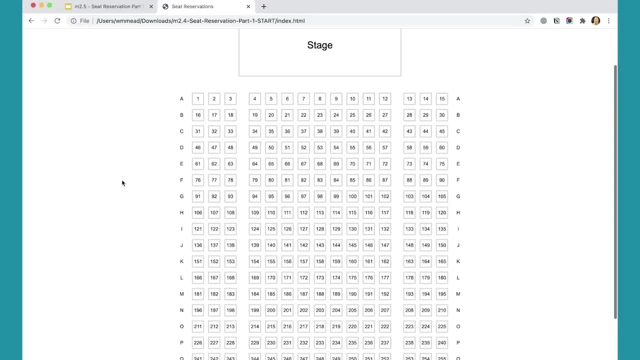 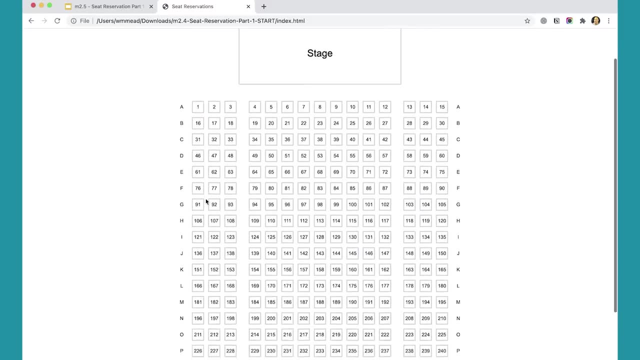 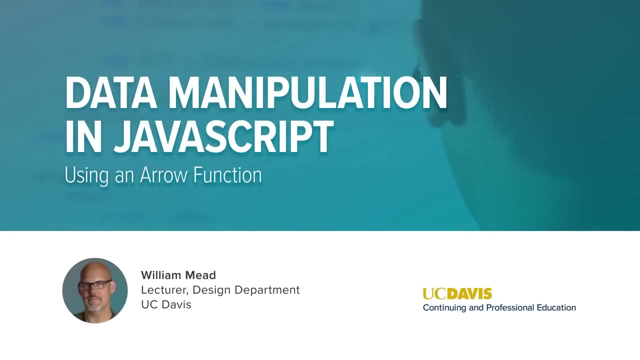 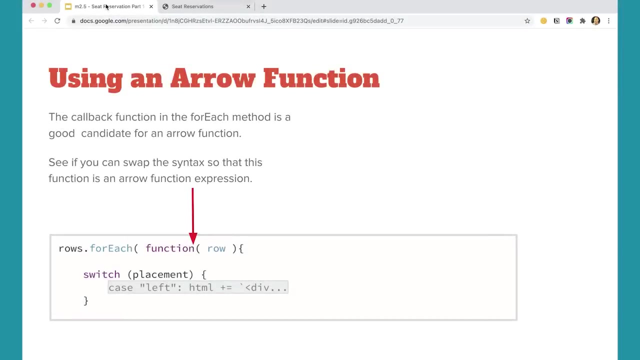 time. now i'm getting the right numbers all the way down to 300, all the way down to 300, and that's working perfectly. in the last video we got our function working. we got it generalized so that we can use one function to create all of the different sections. 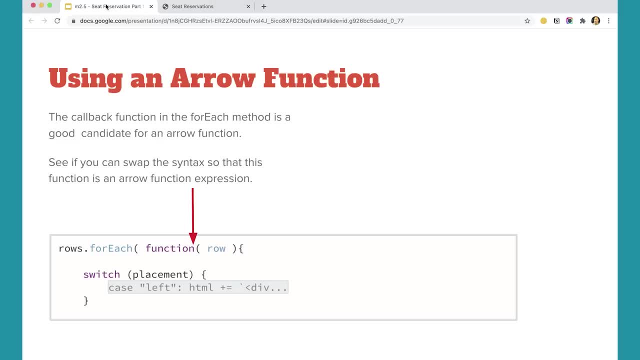 for our seating chart and that's great. and we ran into a few problems along the way, which is normal, and you know you make mistakes- i make mistakes too- and you just have to trace, trace them down and you just have to go back and fix them and see if you can figure out what's. 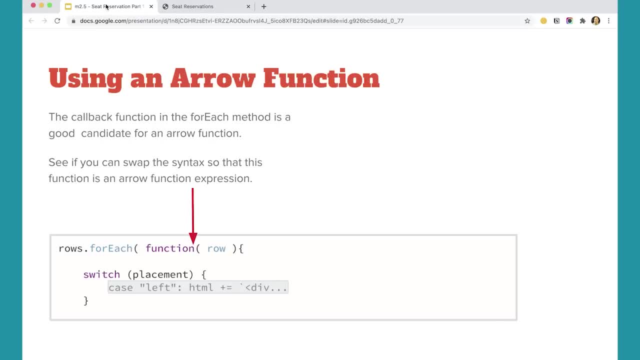 going on, and that's part of the process. it's part of the process of programming with javascript, and this is not a terribly difficult function, but it's. it was. we had done a lot with it before testing it. so, um, you know there's likely going to be problems that you need. 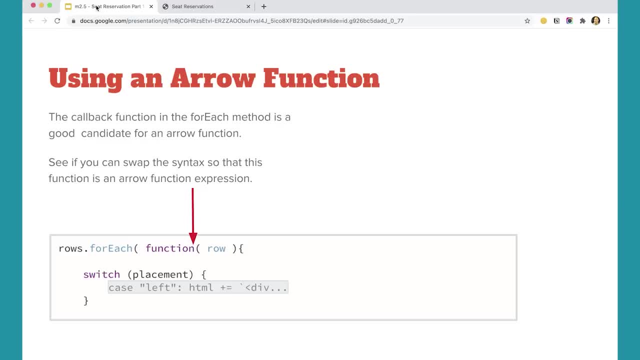 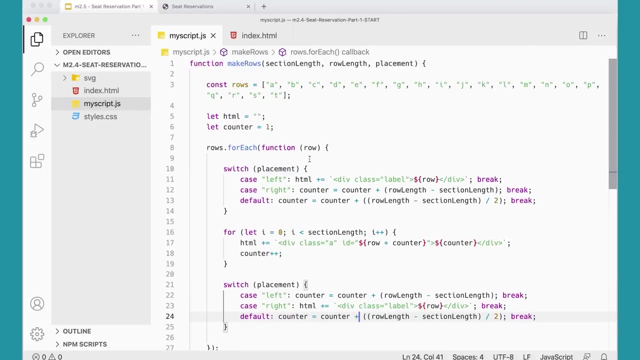 to sort out. next, we can look at using an arrow function and swapping this out for an arrow function. we talked about that before, but now's a good time to go in and say, okay, we've got our function here. this could become an arrow function, which means we have the equal. 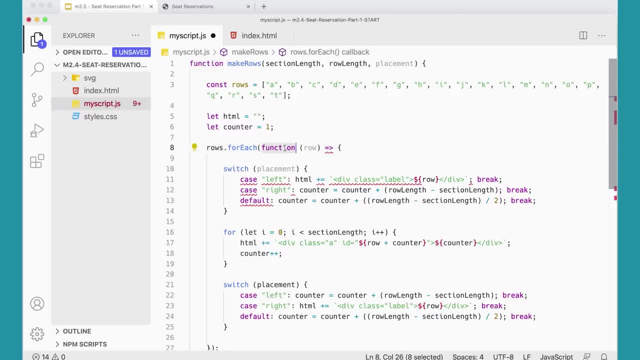 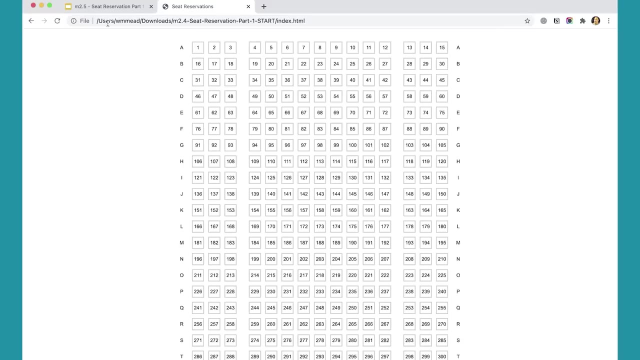 sign. so if you haven't done this already, you could do this: get rid of the function word there and then, because there's only one parameter here, we can just have row and there we go. so that should work exactly the same way as before. just test it and make sure that it does. 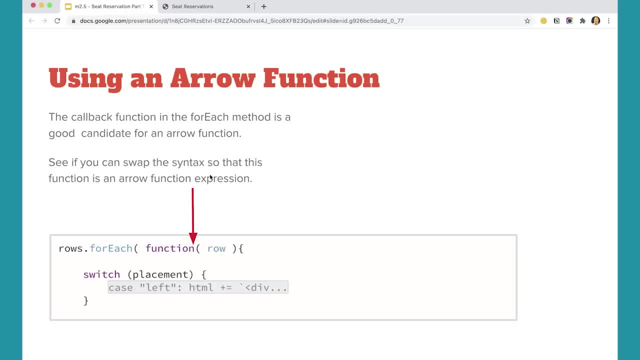 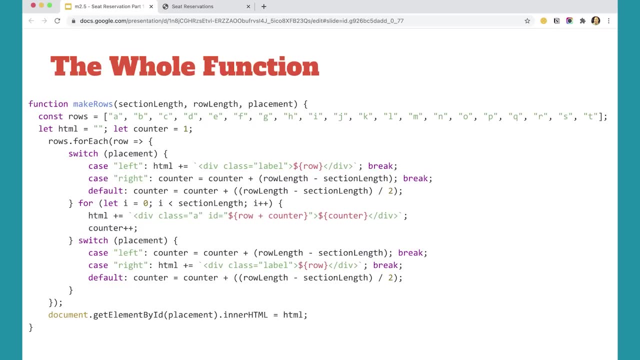 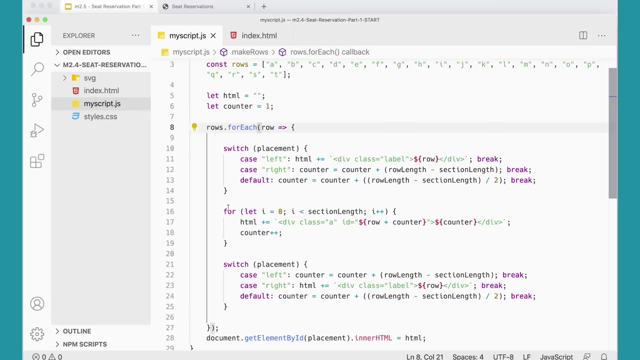 and that gives us our arrow function, which is kind of a nifty thing. and here's our whole function. let's go take a quick look at it in the code editor over here so we can really scroll through and sort of see everything we're testing, we're looping. 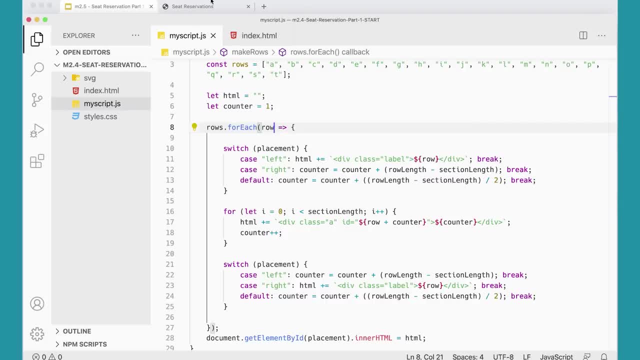 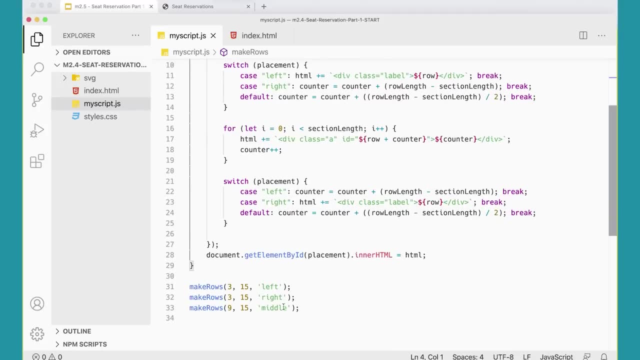 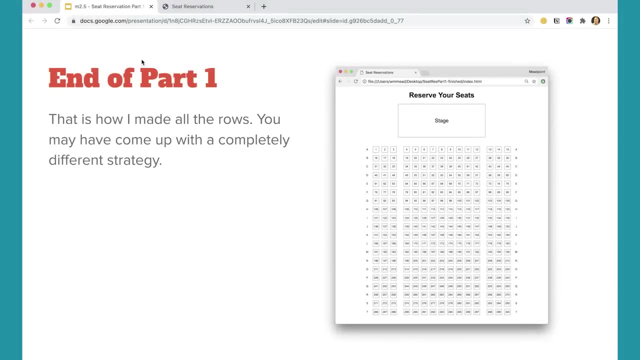 and we're testing and adding these elements, and then we actually run the function three times to create the three sections. we've reached the end of part one, which was just creating the interface, creating the seats that we need in order to make our little web application you may have. 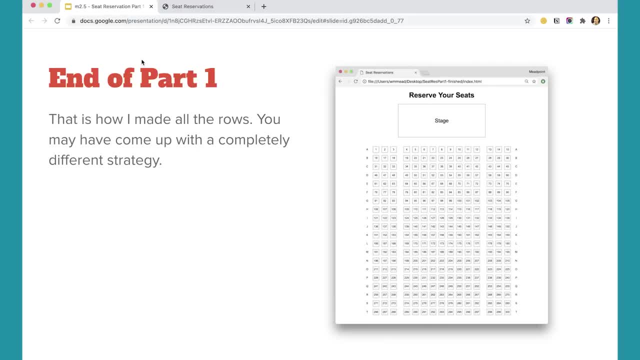 come up with a different strategy, but this was the strategy i came up with for solving it, and there may be other ways or other ways of laying out the seats or doing other kinds of things, and that's totally fine to have a different way of doing it. 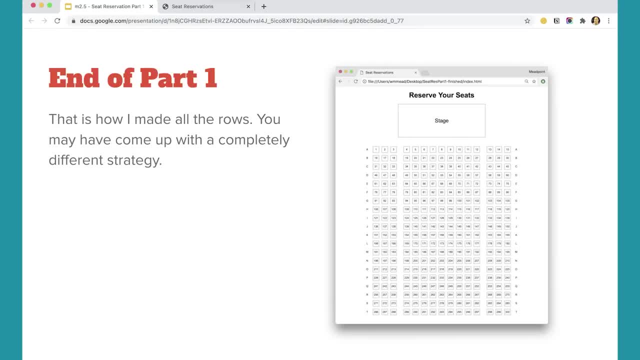 or you may have gotten part of the way done and that's fine too on your own, and that's totally fine. the best way to learn this stuff is to just sort of take on the challenges and practice at it and see if you can get it for the next. 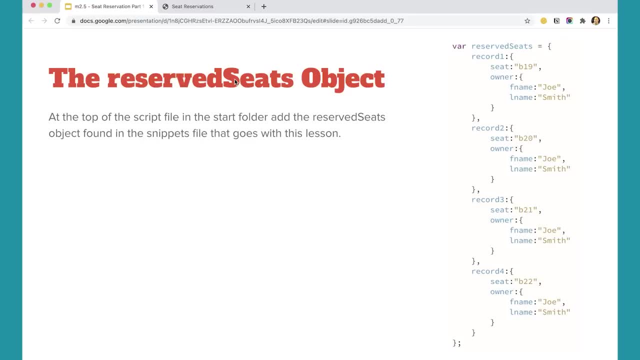 challenge the next part. we're going to add a object at the top of the page, the top of the script file, and this object is going to be similar to the type of thing you would get if you were going to the database, to a database, to get seats. that 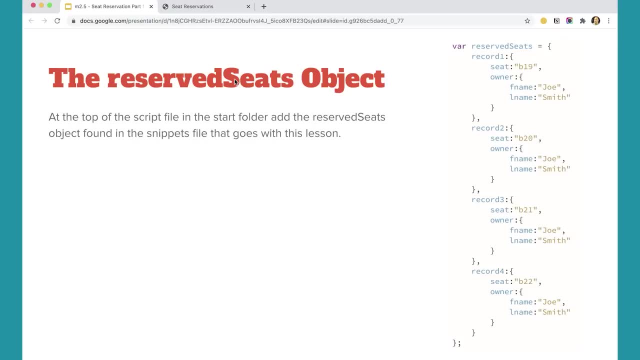 had been previously reserved, so we want to add this object to the top of our document. here. i will provide you with a snippet that includes this piece of code, so you don't have to type it. it's kind of annoying to type. you could type it if you wanted to, but 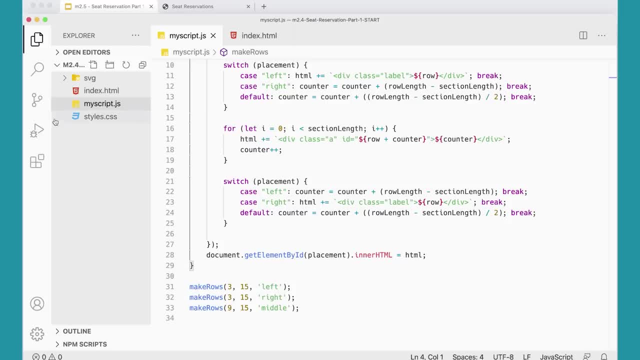 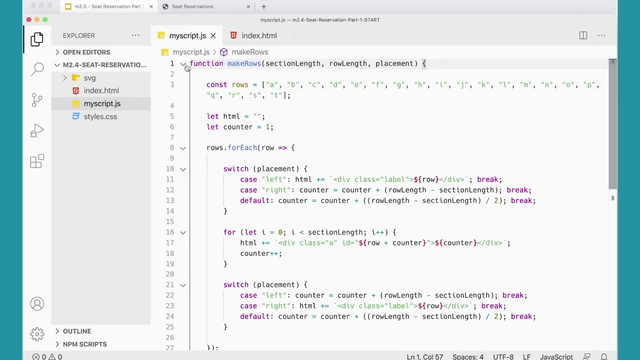 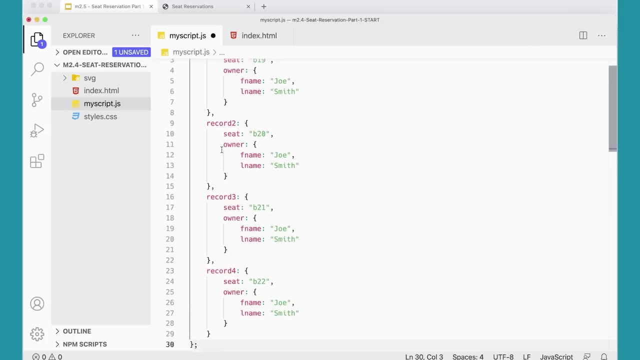 i will provide you with a snippet and you can just come in here and paste that right at the top of the script file here. just move that down and just paste it in here and again. this is going to be as if there were some seats that had been already. 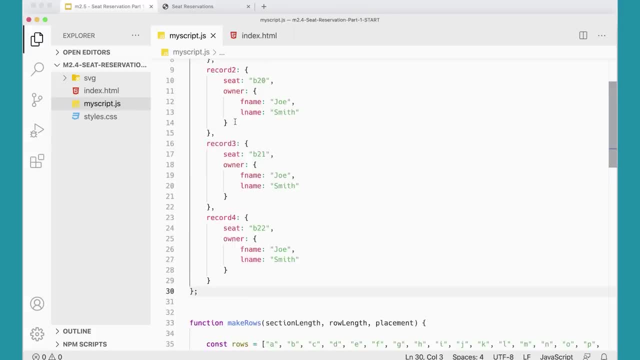 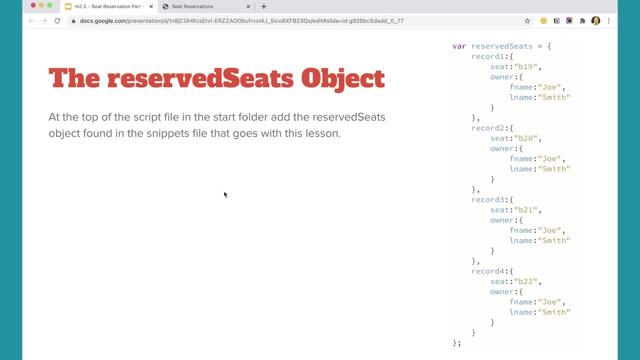 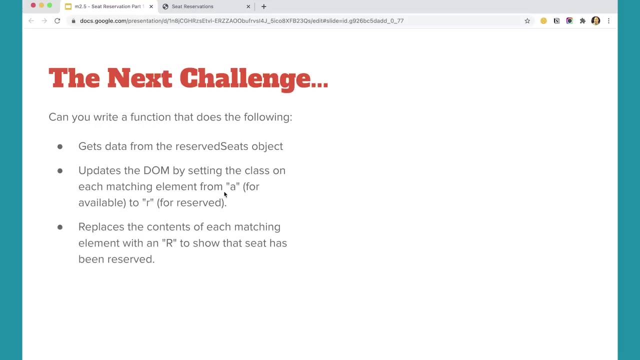 reserved and we'll handle that in the next part of this lesson. and if you want to take it on as a challenge, what we want to be able to do here, see if you can do this, take some time and see if you can do this challenge without. 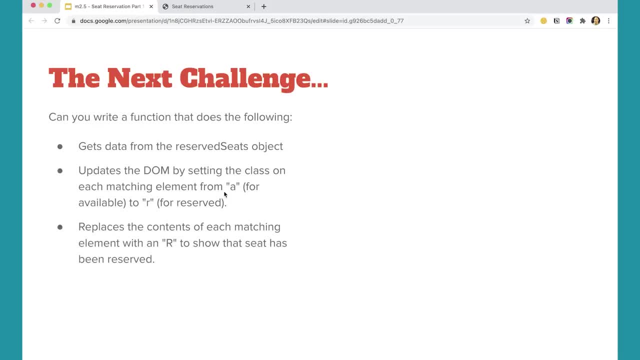 going forward from here with my videos to see how i do it, because you'll learn a lot more by trying it and even if you try and fail, you'll learn a lot more about javascript that way than you will just by running through my solutions. but what we want to do is: 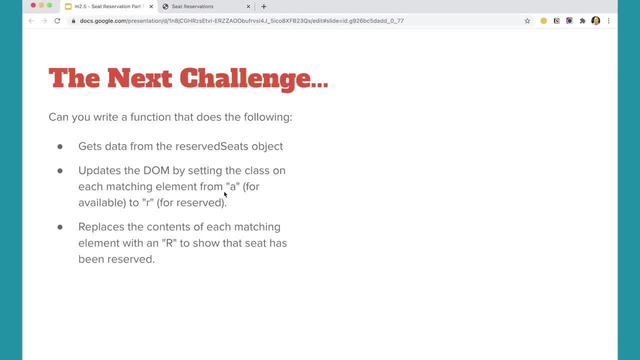 go into that object and get the data from the reserved seats object and then update the dom by setting the class on each matching element from a for available. remember that's why we put that class on those seats to r for reserved, and i already have the styles and the 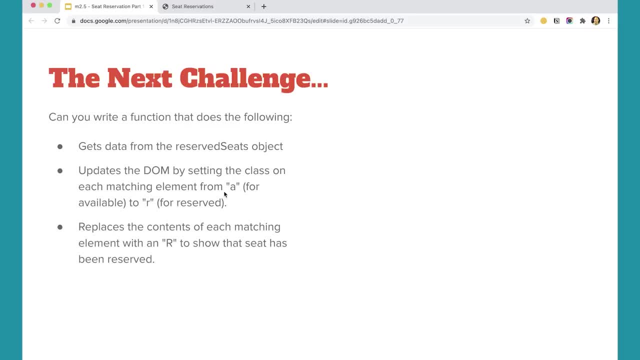 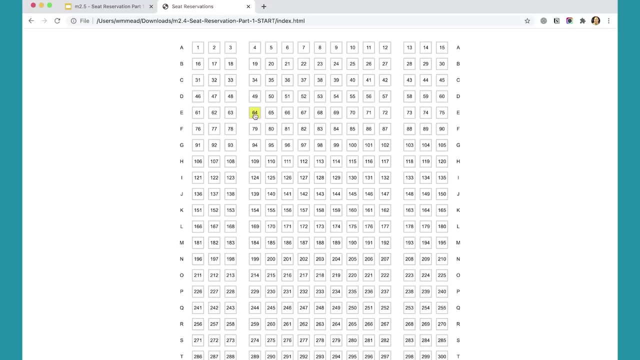 stylesheet to handle this, to handle these two classes. you'll see they're on there and then you want to replace the contents. currently, the contents of the seats are the numbers of the seats. that number matches the id number. we're going to replace that with an r, if it's. 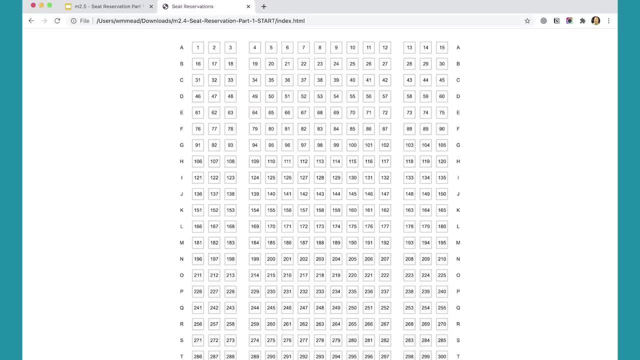 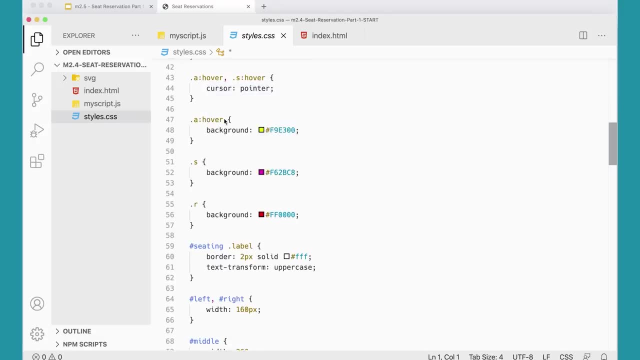 already been reserved and you'll see, if you look in the stylesheet over here, that i have some styling for a s and r different background colors. so this, the styling, is there already. you don't need to worry about that. but see if you can get, see if you can write a function. 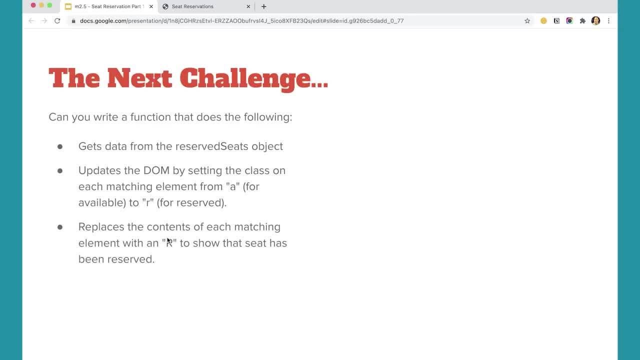 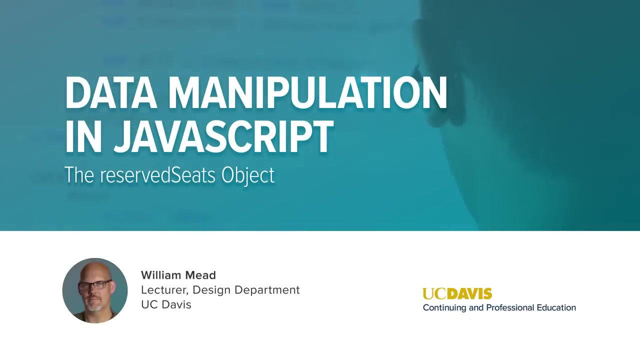 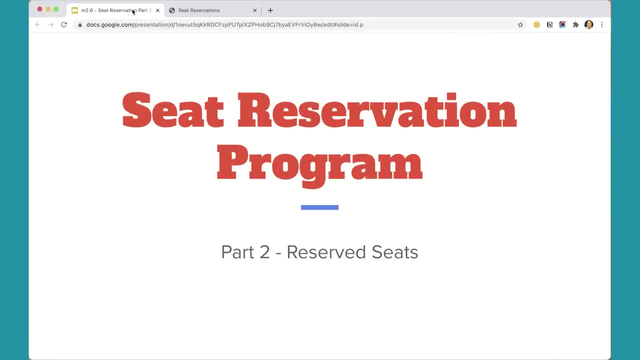 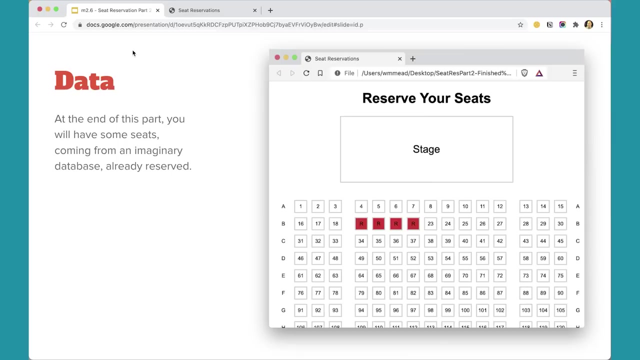 that goes and gets the data from from that object that we pasted at the top of the page and changes the dom to show that those seats have been previously reserved. seat reservation program part two, marking the reserved seats for this particular part of the project. we're going to take the data. 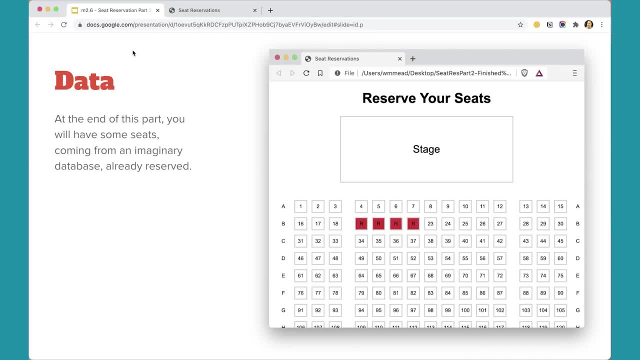 that we had up at the top of the page and use it to mark the seats that correspond with those with that data as reserved. the styles are already on the stylesheet. your challenge was to take the take that data and then use it to find those seats and change the class. 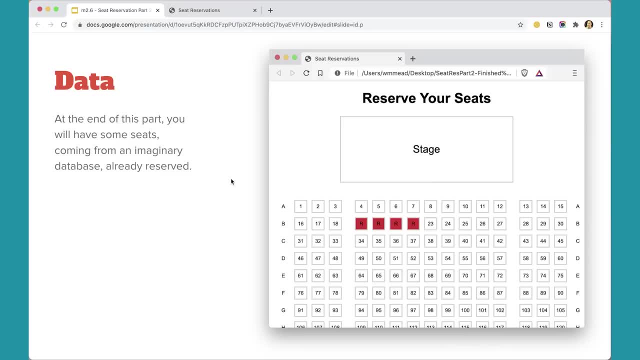 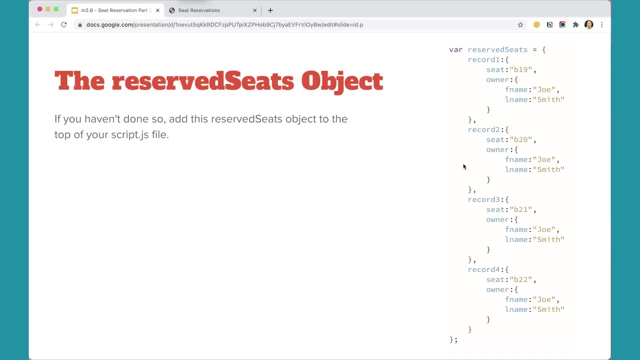 from a to r, and hopefully you were able to do that and we'll see if my solution for this was different from your solution for this. if you have not done so, make sure you've added this object for reserved seats up at the top of the page and this object. 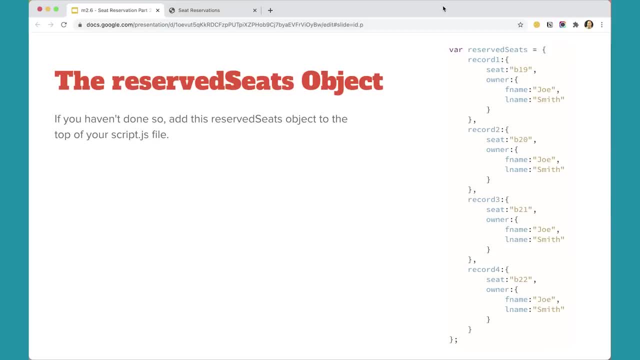 is just. it just looks like a a piece of data that you might get from a database. we're imagining that we had a database in the back end and that that data is being saved in the database of previously reserved seats and we need to be able to. 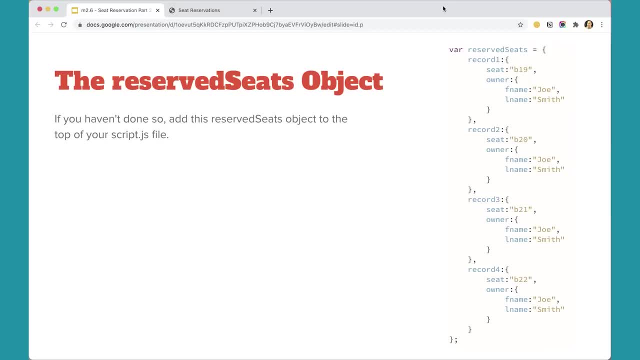 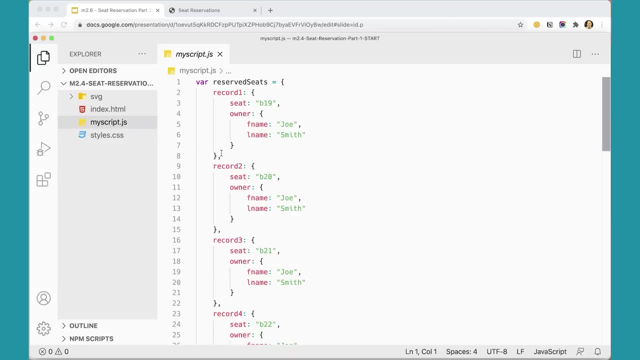 know what those seats are and that data would usually come in at the top of the page. so we're going to use the json string javascript object notation, and then we would use json parse to parse that into an object. but here i've given you the object already, so you can just add it. 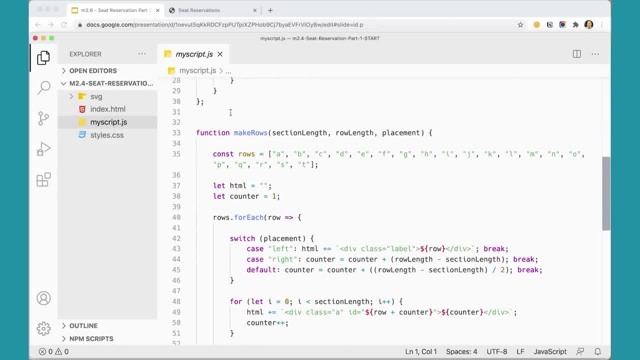 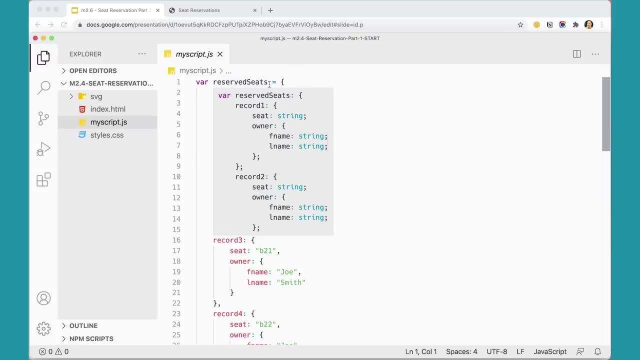 to the top of your page here and you can see that i have it on my script file just before the make rows function that we did in the first part. so that's all in place and ready to go. the first thing that we could try is a. 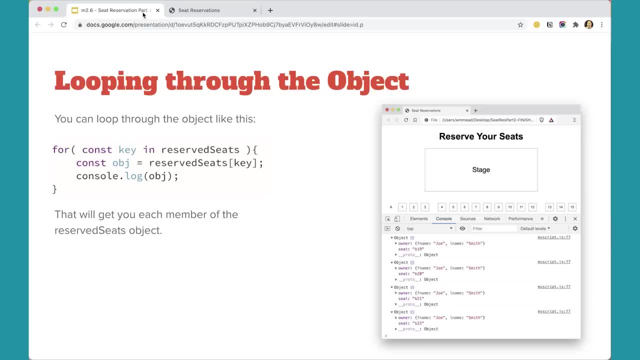 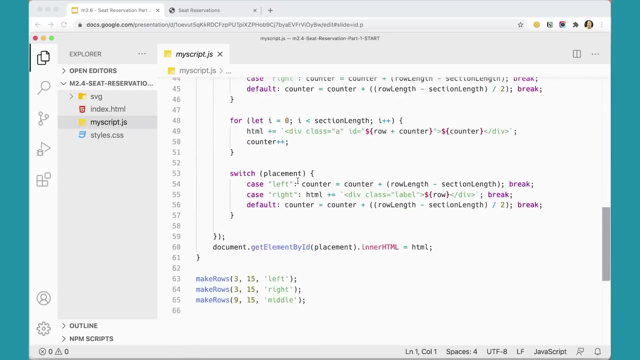 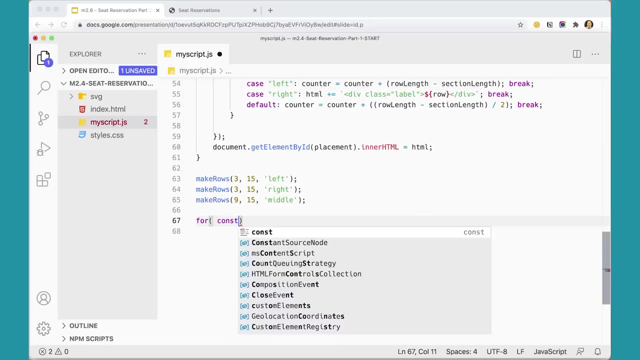 for in loop which allows us to loop through objects to see if we can access the the different pieces of the object inside that reserved seats object. so let's try that real quick. so down here i'm just going to add a for loop for const key in. 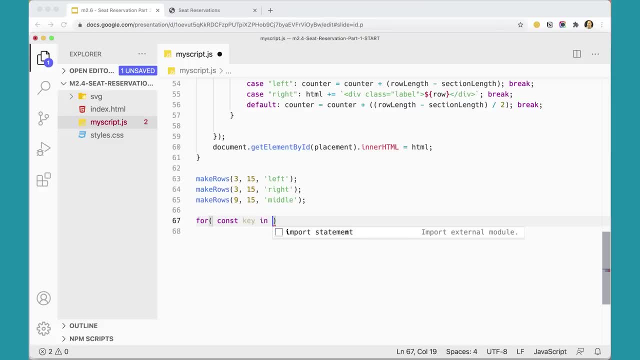 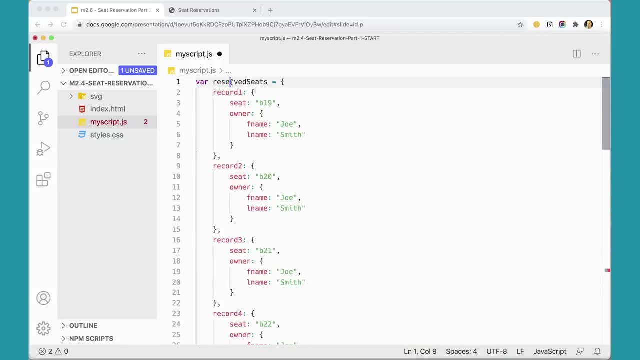 for object to to do. what is it? what's the name of this object up here? reserved seats, key in reserved seats, and all i want to do here is just see what i can get out of that. i'll make a variable const. object: obj for object object. 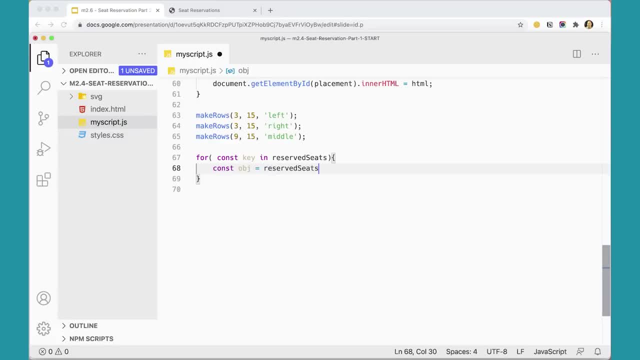 equals reserved seats, square bracket key, and that should take each key in this reserved seats and put it into this variable object. and then what if we just console log that object up, console dot log obj, to see what we get? so over here i have the file open. 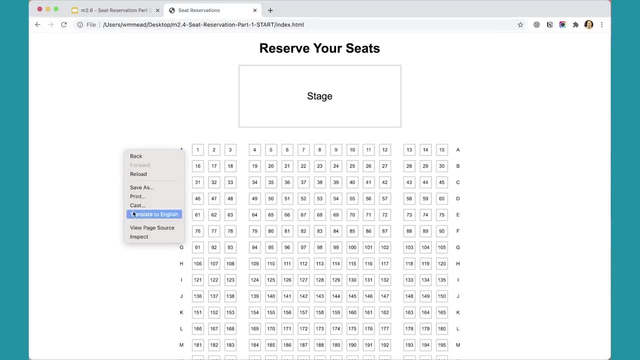 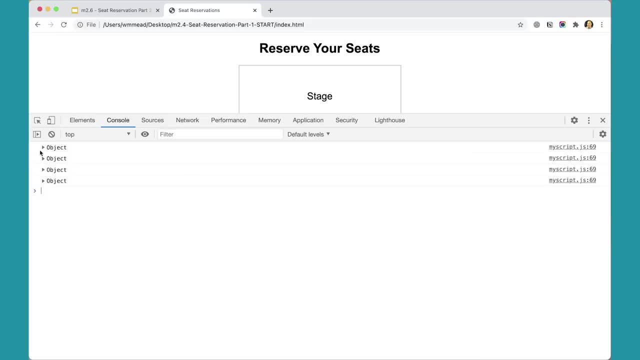 and i can refresh it, and then i can choose, inspect, get rid of this thing, and if i click on the console you can see i'm getting those objects with all the information. now i want a particular piece of information. how about the actual seat? so what happens? 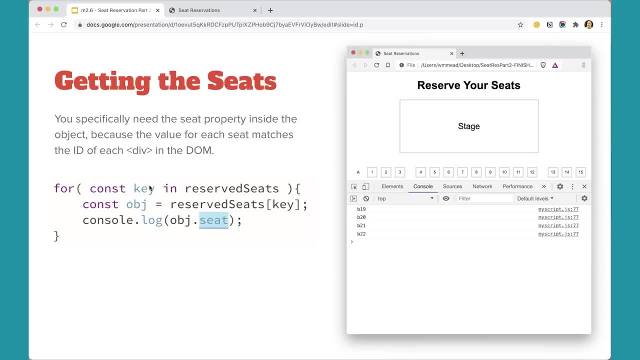 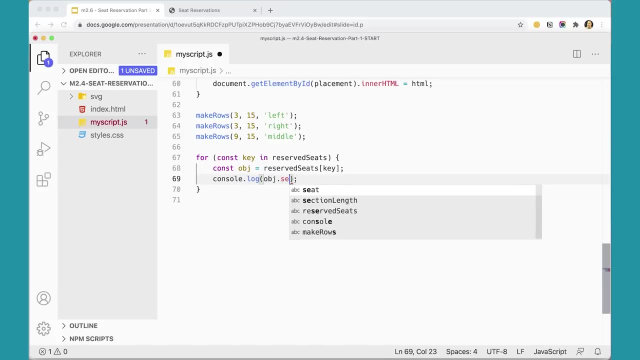 if i go back and change this so that i'm just doing object dot seat just to get that one object and that's should get me my seats. so let's see if i can do that object dot seat so you can see that i'm using this sort. 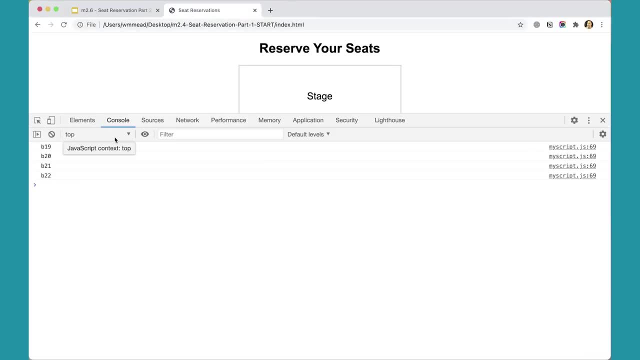 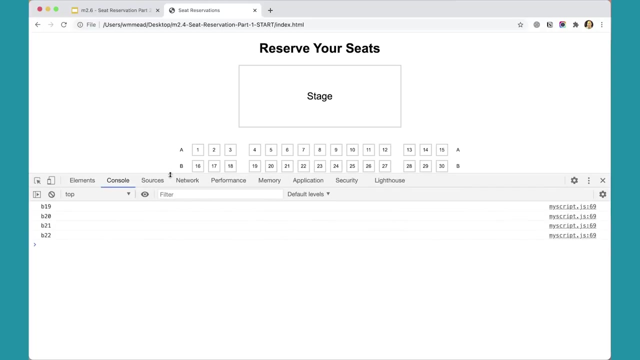 of step-by-step process to figure out how i can get to the data that i want to get to inside of my object. this is a good way of playing with javascript to help you try to understand how to access data within an object like the. Sometimes you have to play around with it a little bit to sort of figure out exactly where to go, and that's totally fine. 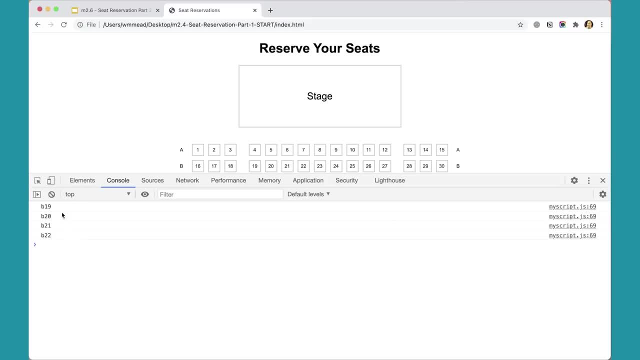 Okay, great, So I'm able to get the individual seats inside of here, and that's what I'm going to need to do to sort of figure out. Now that I've got these seats, I need to use this data to go into my DOM here and mark 19,, 20,, 21, and 22 as reserved. 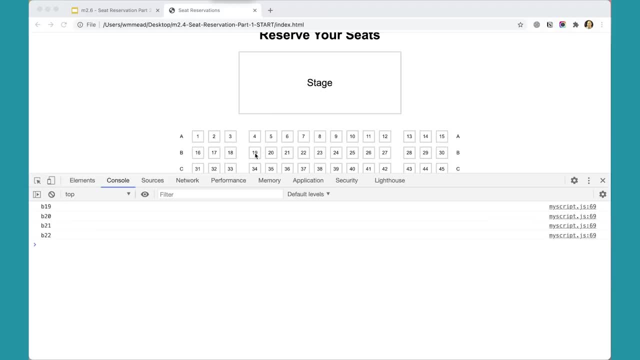 To do that, I need to change these seats. I need to change their class from A for available to R for reserved. That will change the color. And I want to change the HTML inside of these, from the 19,, 20,, 21, and 22 to just a capital letter, R, to show that they're reserved. 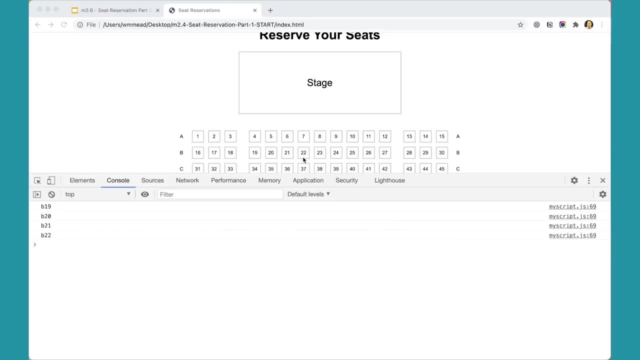 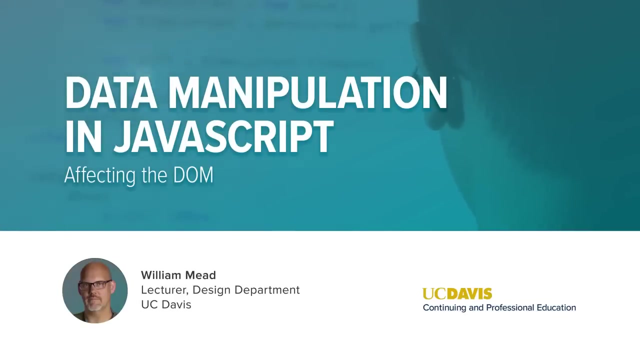 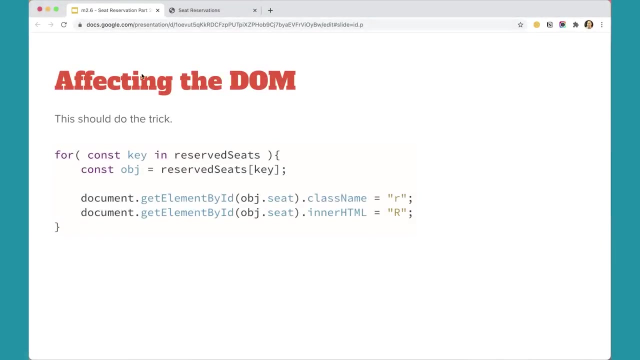 And you should be able to do that. See if you can actually write the script yourself without going on to the next video. Okay, Okay, Okay, And see if you can get those two pieces of information in there. Hopefully you were able to solve that little challenge and come up with something like this. 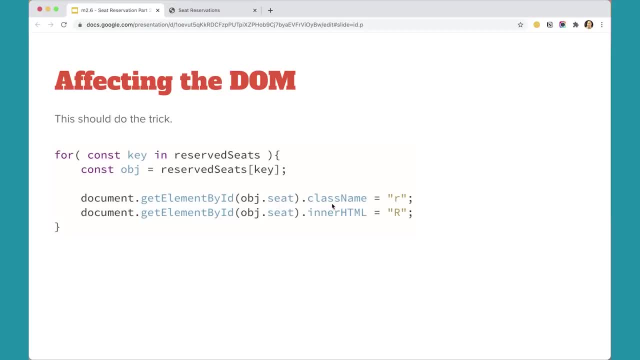 Document. get element by ID objectseat, set its class name property to R, and then we're setting the inner HTML to R. So that's a pretty straightforward way of doing this And hopefully you were able to get that. But let's put that in here. 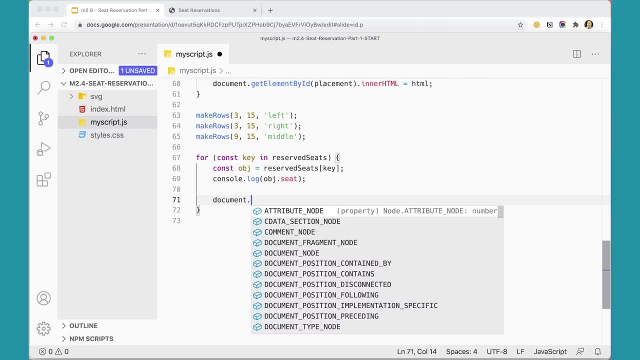 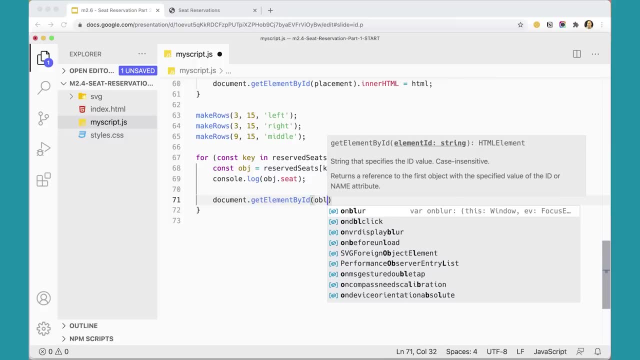 So I'm going to come down here and do documentget element by ID objectseat. Now we know that that's going to as we loop through, it's going to be B19, B20.. And those are the IDs in the page. 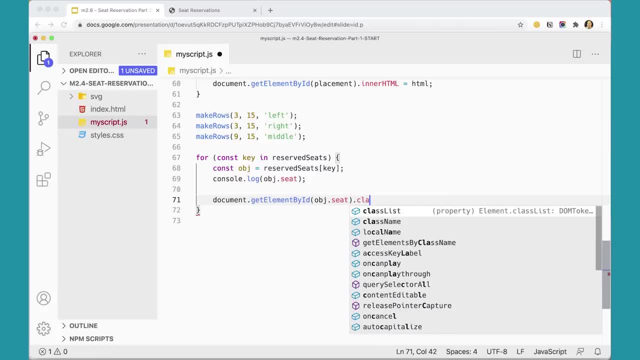 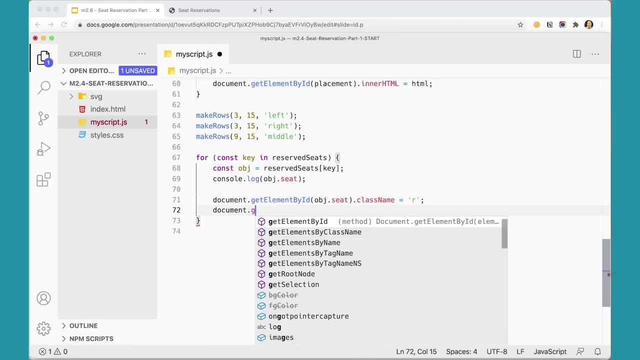 So we know that classname equals R, And then documentget element by ID objectseatinnerHTML And set that classname Equal to just a capital R, Like so, And it doesn't matter if you use double quotes or single quotes. 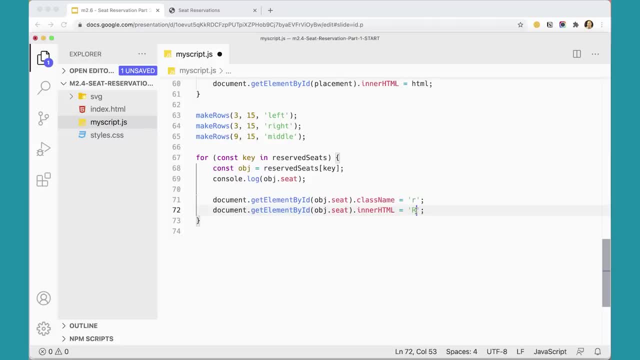 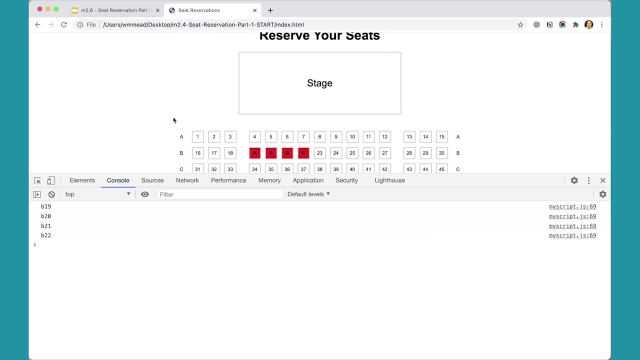 I guess just for consistency, I'll keep it single quotes. There we go, And if I go over and test this, you'll see it's working. It's going in and getting those seats out of that object and setting them to reserved. 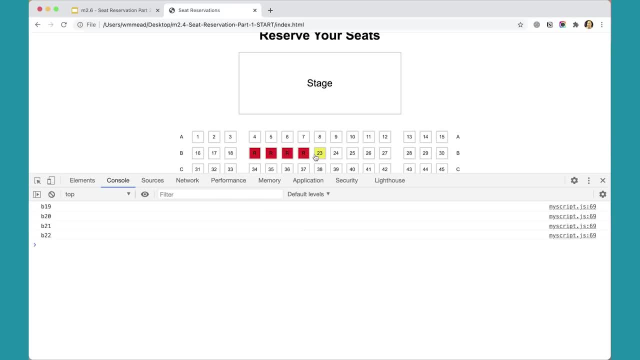 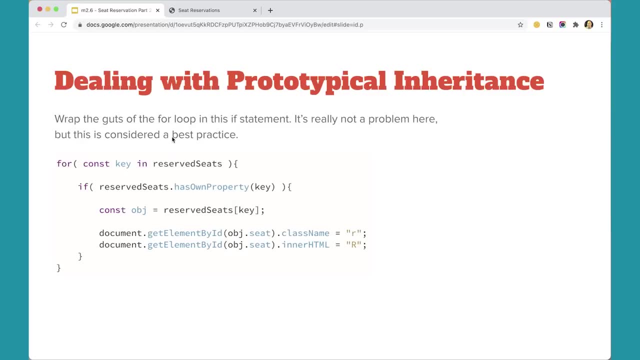 And that's great. There's a few more things we want to do here Just for best practices, And that is, specifically, we want to wrap it in this if statement, just to make sure that we're working directly with the properties in this object. 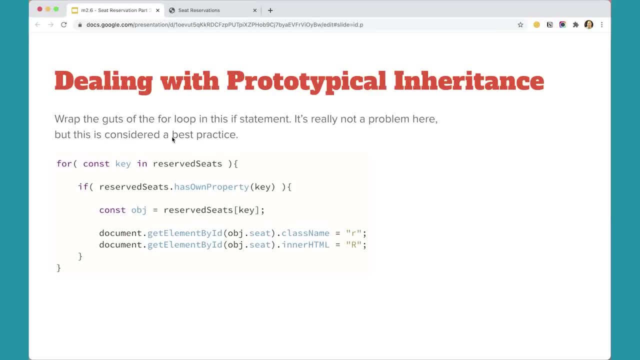 And not something that these objects inherit from further up the prototypical chain. Now, these objects aren't going to inherit this from further up the prototypical chain, But this is considered a best practice To make sure you're dealing with the properties directly on the objects rather than something that's inherited. 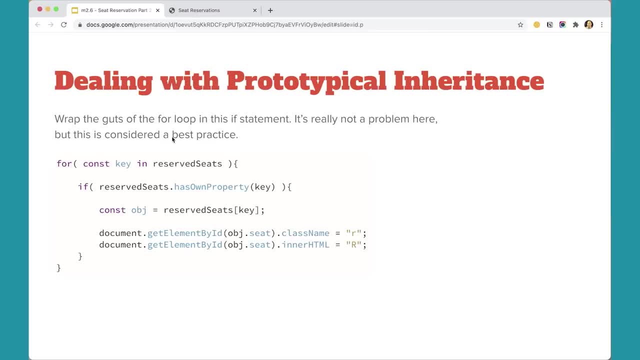 And part of the reason why we went through that piece earlier in this course on the prototypical inheritance was specifically so that this piece of this project would make sense And that you would understand that objects can inherit properties from further up the chain, And we don't want that to happen. 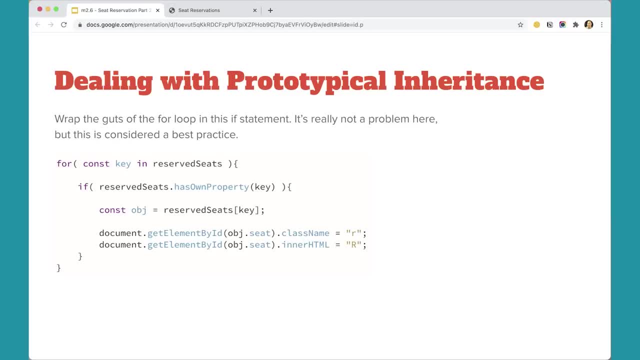 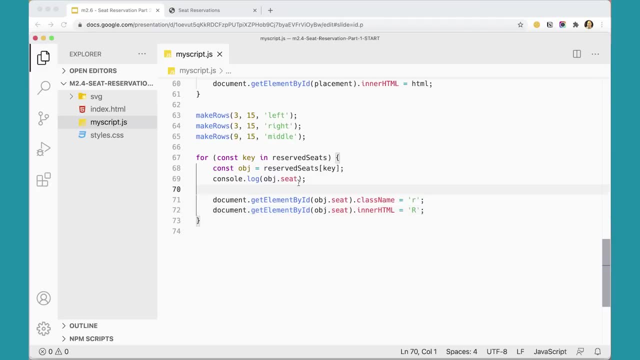 So let's go ahead and just add this if statement in here And make sure that all works well. We don't need to console log this out anymore, If, If, I can just take all this stuff and stick it in here And 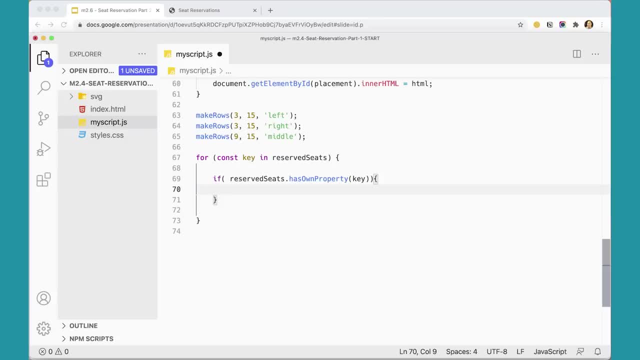 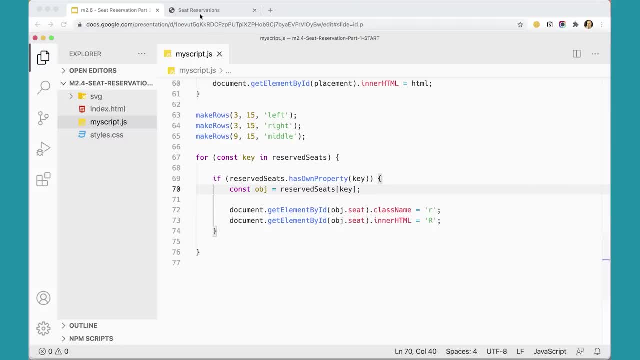 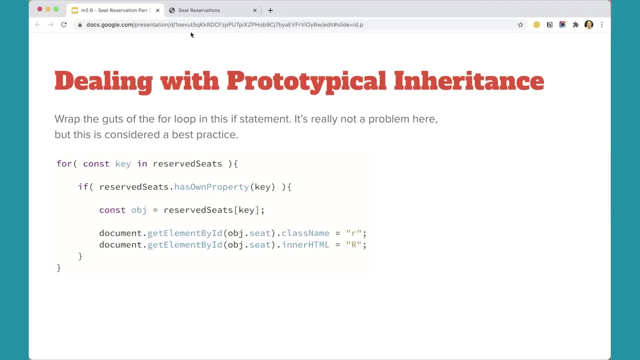 Because we just don't need it here. That shouldn't change any actual results over here, But we can just go test and make sure that it still works. I didn't type anything wrong And Yeah, that's. That's just a good kind of check, right there. 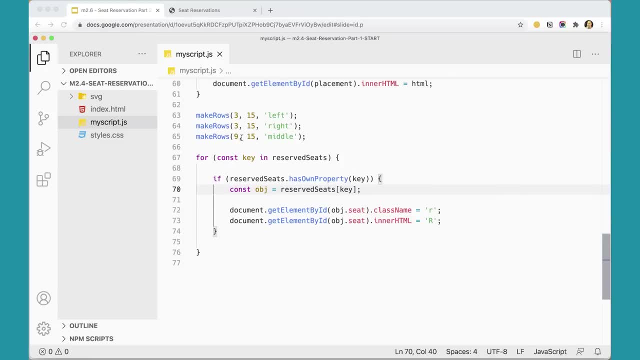 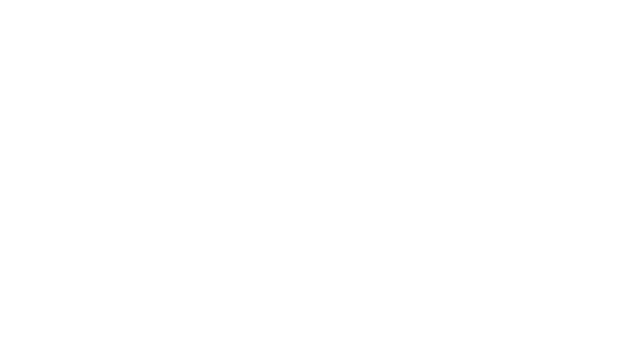 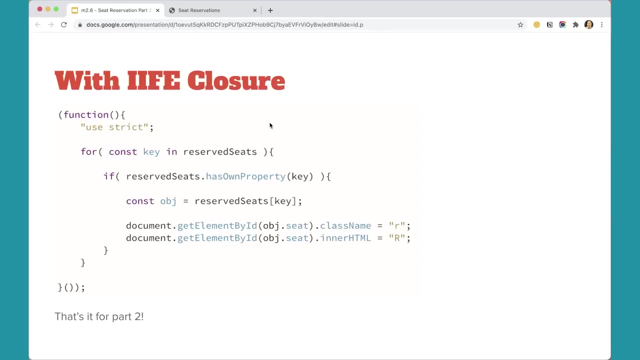 Yeah, Yeah, Yeah, Yeah, let's do that, OK, great. So this is the. this is the basic piece that we need here. Let's just do a few more things for best practices, Yeah, And then the last thing we need to do is wrap the whole thing in an enclosure. 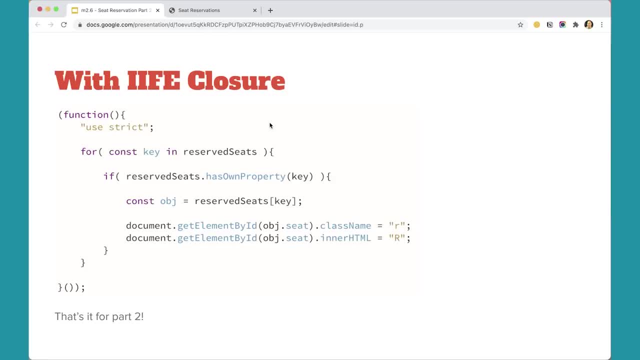 An enclosure And the, the, The immediately invoked function, expression closure. So let's do that, We'll do that in the next video And And sort of wrap up up this part and get ready for the challenge for the next part. 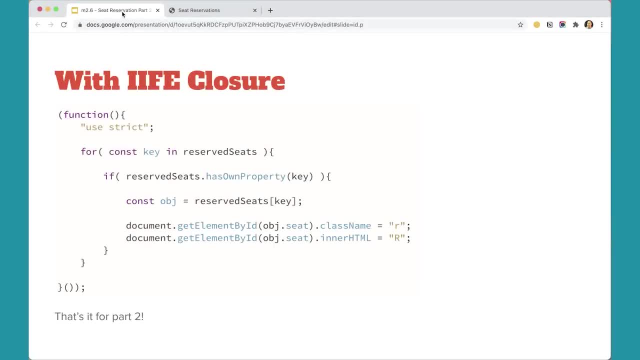 Next, we'll add the IIFE, the immediately invoked function expression, and put it around our for loop, just because we don't want this for loop hanging out in the global scope. And it's worth mentioning that this is a really good use of the IIFE. closure. 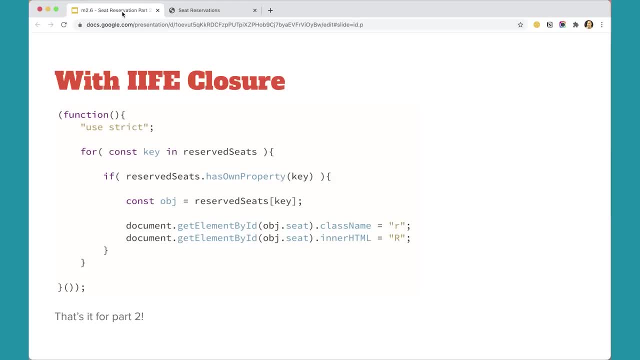 the immediately invoked function expression closure, because there isn't really a reason to create a named function for this for loop, And not only that, but everything else that we're gonna do for this project is gonna go inside of this closure, So it's a good idea to go ahead and put it in. 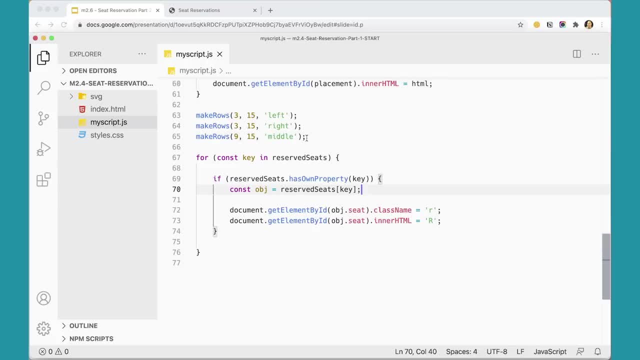 So let's just come back over here and add this. So again, it's a set of parentheses, and then in there we're gonna add a function with its own curly braces and parentheses, and then a set of parentheses just for good measure to do. 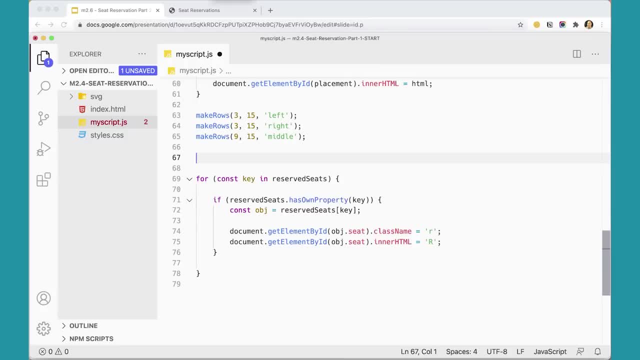 to get that to work right And I did that wrong, So I'm gonna do it again, just to make it really clear. Parentheses function with its parentheses, its curly braces and another set of parentheses to make it run. There we go like that. 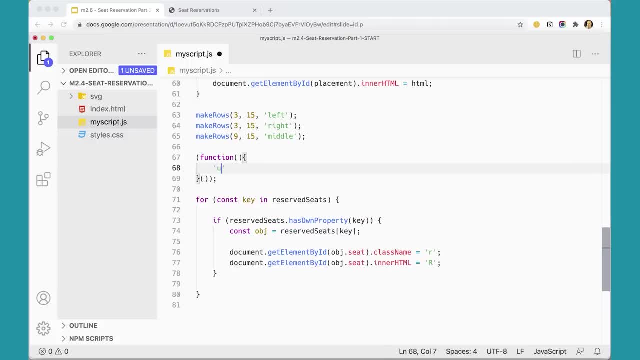 And then we go inside the curly braces and we're gonna add our use strict directive there and press return. And then we're just gonna stick all of this stuff, cut it from there and paste it in here, And then that will take care of that. 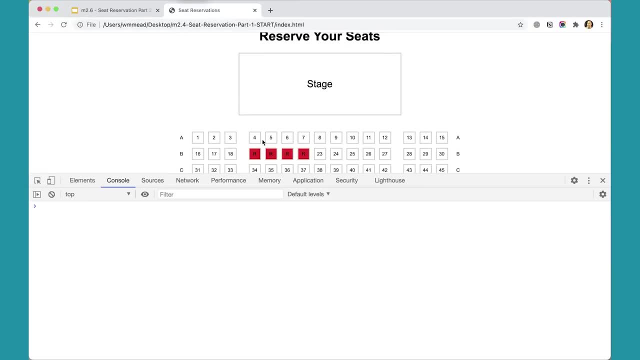 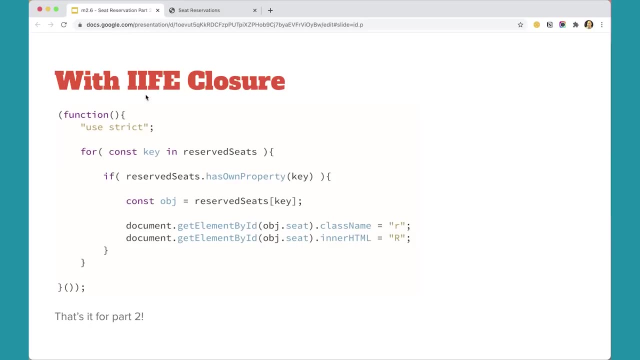 And again, we can check over here and make sure that it's all running right, that I did that right and I did So. that's all working. that's fine, Okay, great. So we have our IIFE, our immediately invoked function, expression. 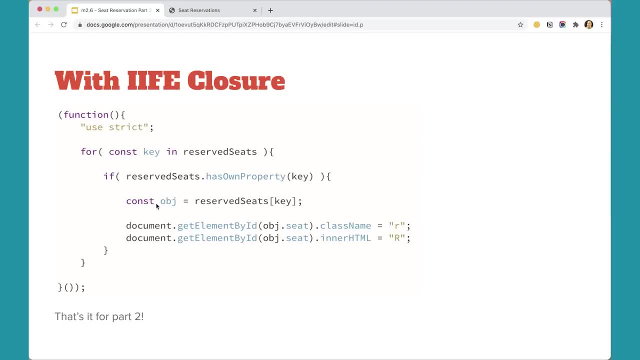 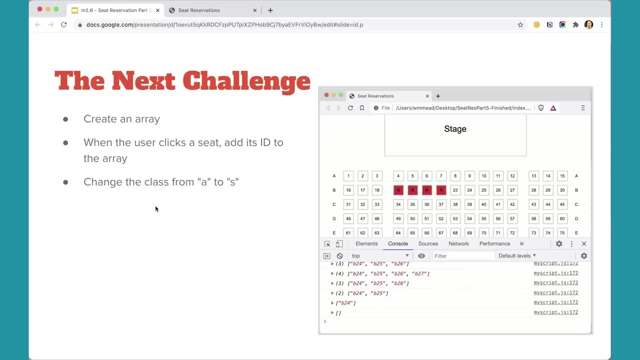 and we have our loop inside of it and we're set to go to the next challenge. And as for the next challenge, this is your next challenge to try to figure out before going on to the next challenge, The next part in this lesson. 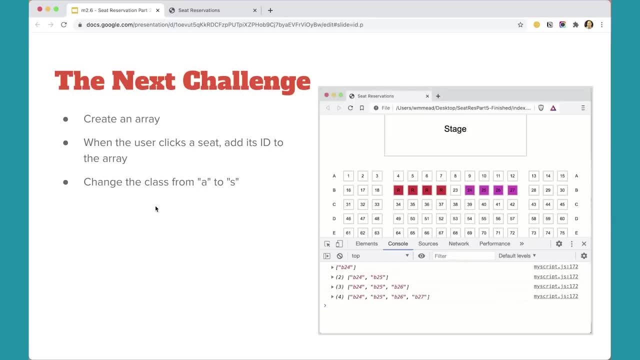 which is we need to create an array And then when the user clicks on seats in the array, when the user clicks on seats, they get added to the array, as you can see down here in my animated image here that the seats are being added here. 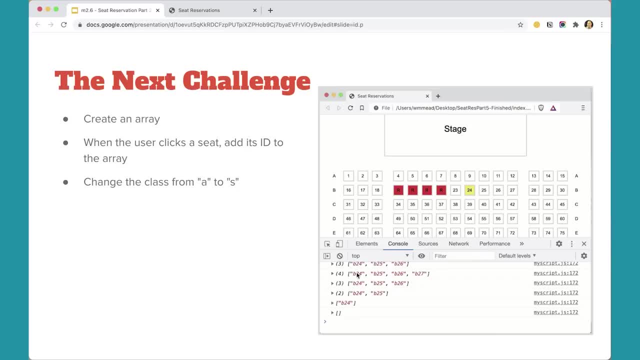 as you put them in, as you click on them, But then, when you click on them again, it takes them out of the array. So see if you can figure out how to do that on your own. That's what we're going to be doing. 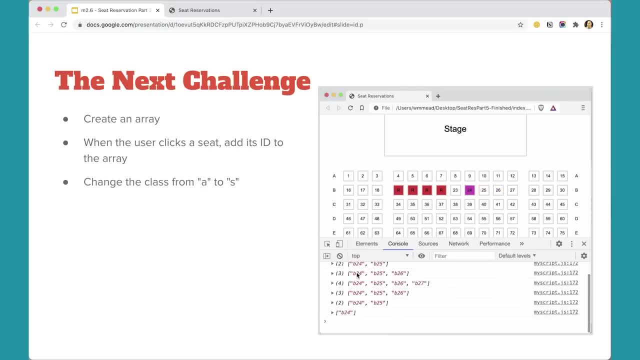 in the next part of this lesson. in part three of this lesson is creating this array and making it so that when the user clicks on seats, they go into the array And if they click on a seat that's in the array, it takes it out of the array. 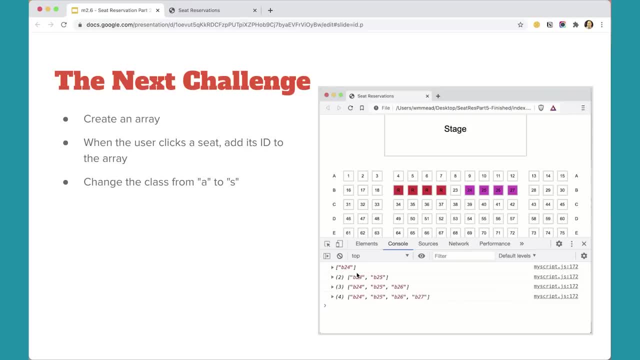 Ultimately, the long-term goal is to: when the user clicks on these seats and puts them in the array, and then they click the reserve seat button, it will save them back up to the object at the top of the page, as if we were putting it back out to the database. 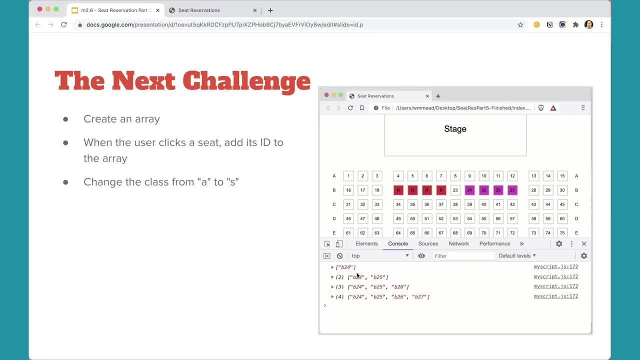 sending it back out to a database, but we'll just be putting it into the object at the top of the page. So those seats are also part of that reserve seats object. Okay, great. So good luck with that And perhaps you'll come up with a different solution. 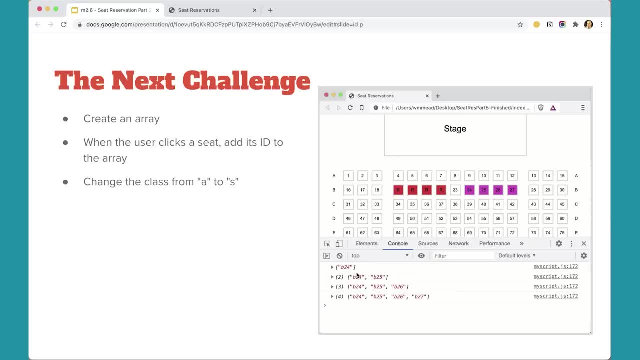 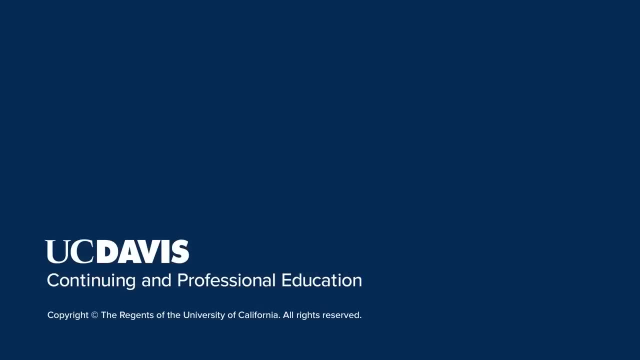 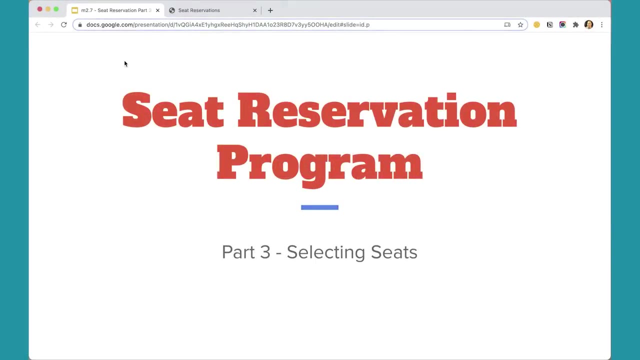 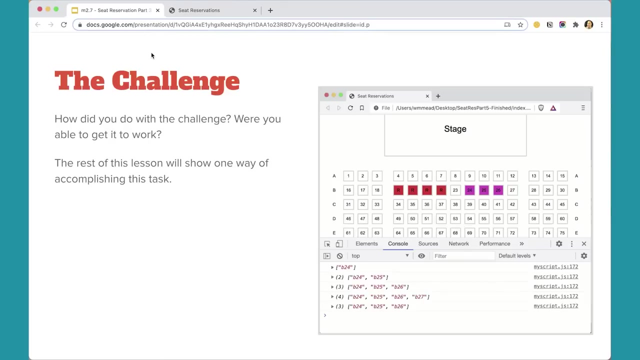 than what I came up with, but we'll take a look at my solution for solving this problem in the next part of this challenge, next part of this project: Seat reservation program, part three: selecting seats. The challenge was to make an array. 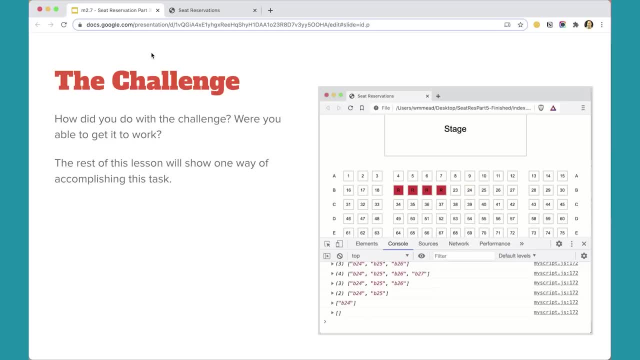 and then make it so that when users click the seats, they get added to the array. If they click the seats that are in the array, they'll get removed from the array. Hopefully you were able to complete this challenge in your own. 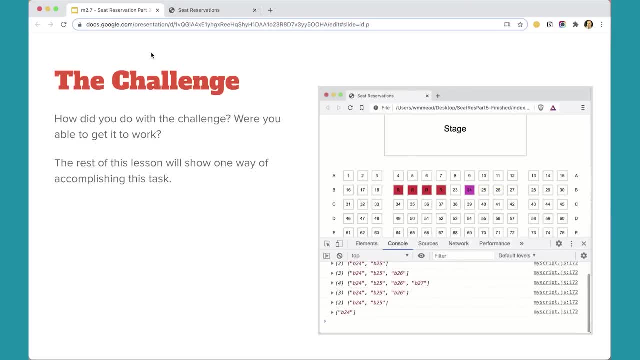 It's definitely a little bit more challenging than some of the other challenges we've had, but it's not super difficult, So you may have been able to do it with a little bit of futzing around. So let's see what we can do with this ourselves. 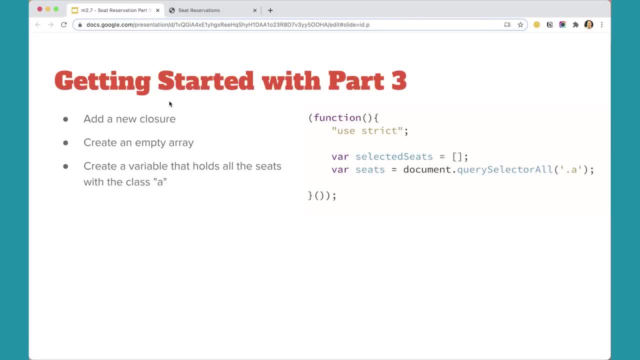 To start with, I'm gonna make a new IIFE immediately invoked function expression And really you could put this in the one that we already have for the for loop. There'd be no problem with doing that, But just to be clear. 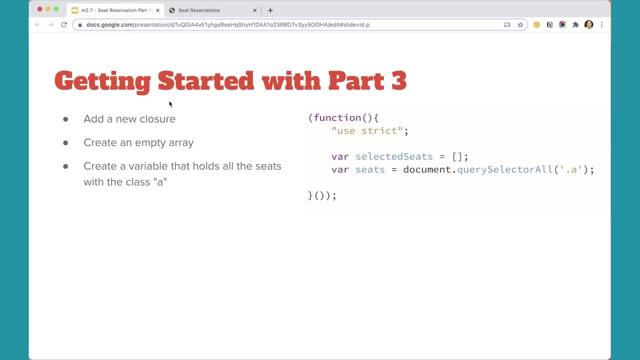 I'm gonna kind of separate it into its own separate immediately invoked function expression and add the two variables: selected seats and a variable for the seats that are gonna go get all of the anchor tags from the all of the available seats from the DOM. 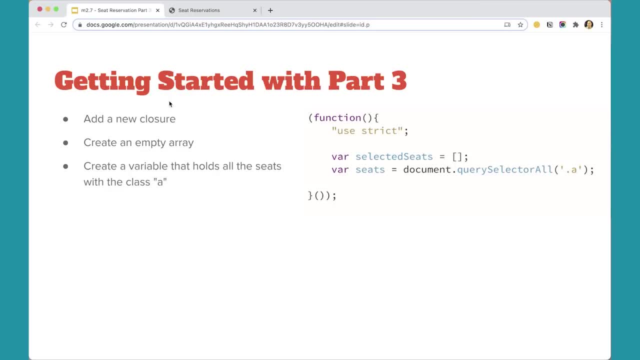 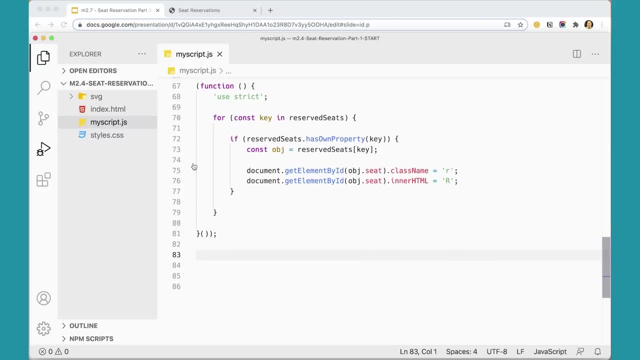 all those divs with the class of A on them, And so let's go ahead and add this over to our script over here. I'm gonna add parentheses and add a function in here with its parentheses, its curly braces and then an extra set of parentheses. 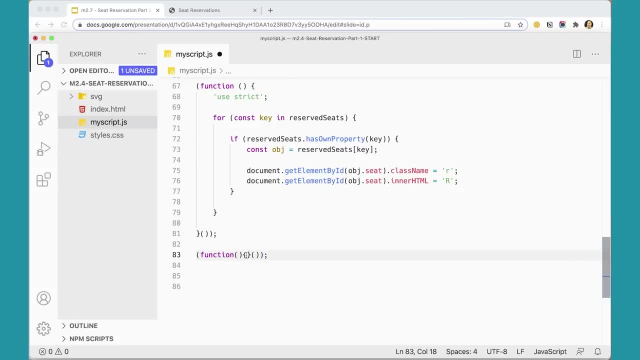 to make it run right away. And in here I'm gonna add use strict And from here I'm gonna create a variable var- selected seats- And you may have created a different variable name, and that's fine, It doesn't really matter what it's called. 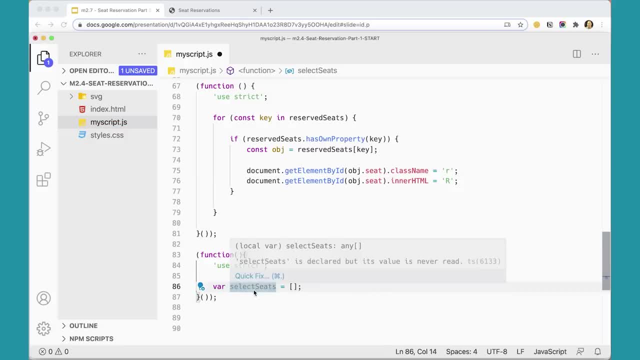 Selected seats seems like a good, yeah, a good, a fairly good name there to use. And then I'm gonna have variable var seats- equals document, dot, query, selector, all, And I wanna get all of the seats with the anchor tag with the class of A. 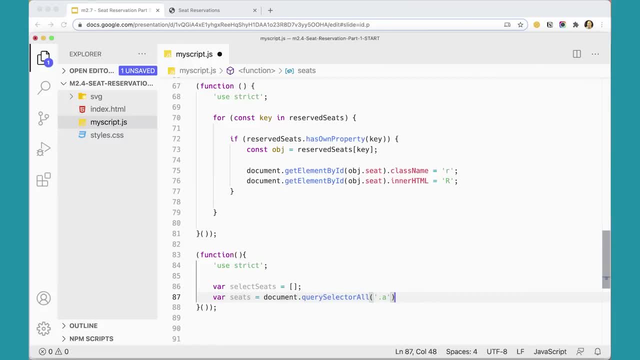 I'm getting confused. anchor tags are A's But we're really looking for elements with the class of A on them, which is the divs with the class of A cause they're available. So they're not anchor tags, but not to be confused with anchor tags. 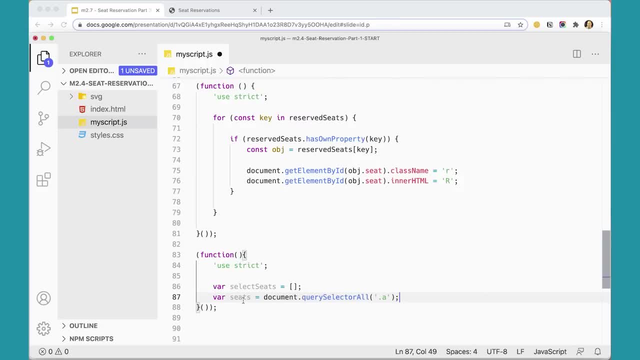 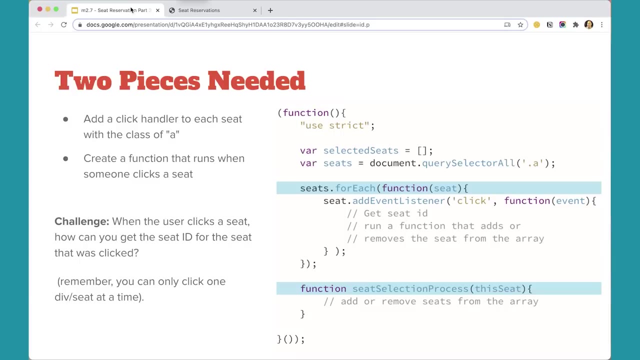 Okay, so that's gonna put all of those seats into this variable. Okay, There, And that will get us ready for the next step here. For the next step, we will need two pieces. We need a piece where we add an event listener to each seat. 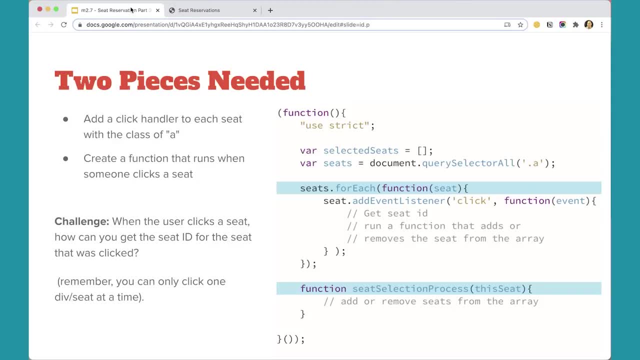 And then we add a function that's gonna run, that's gonna take that seat and add it and remove it to the array when you click it. So we'll do this part in the next video. So let's go ahead and run the event listener. 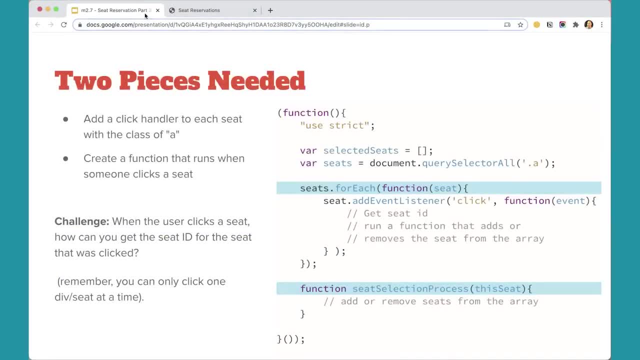 Okay, now we need these two pieces. We need to have an event listener. We need to loop through all our seats and add an event listener so that, when one of them is clicked, we can actually run a function that will add it to the array. 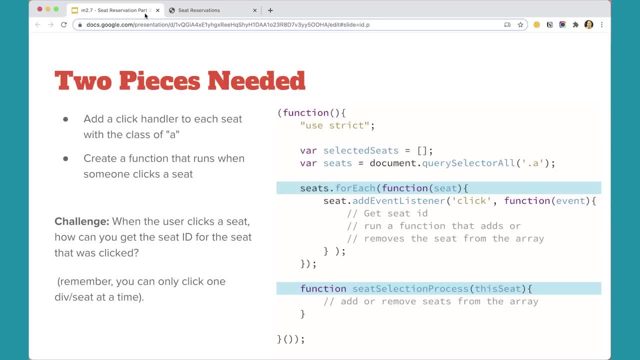 And we could use any number of types of loops here. We can use a for of loop, we can use for loop. I'm using the for each method because I think that's nice and clean and works really nicely with arrays. so i'm going to use that method here. but you could use a different. 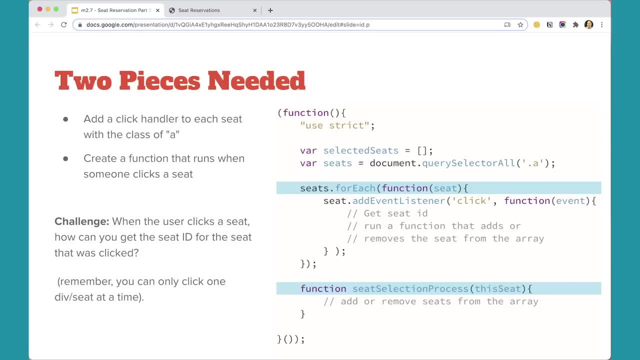 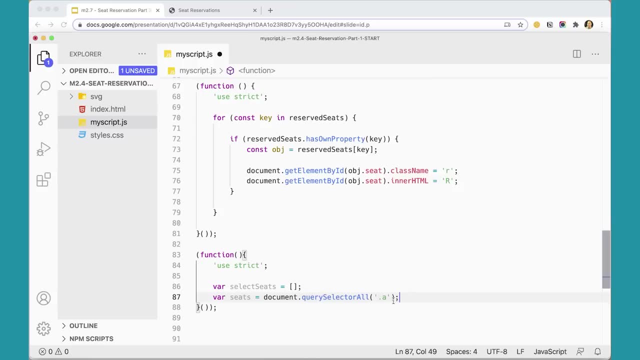 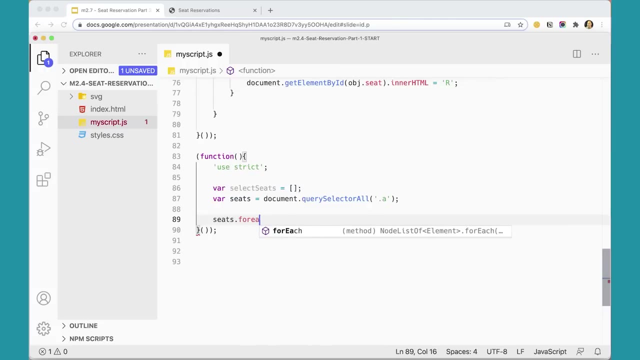 method, or perhaps, when you solve this, used different type of loop to do this, and that would be perfectly fine as well. there's always more than one way of doing things, but over here i'm going to add a a for each loop. here, seats, dot for each. 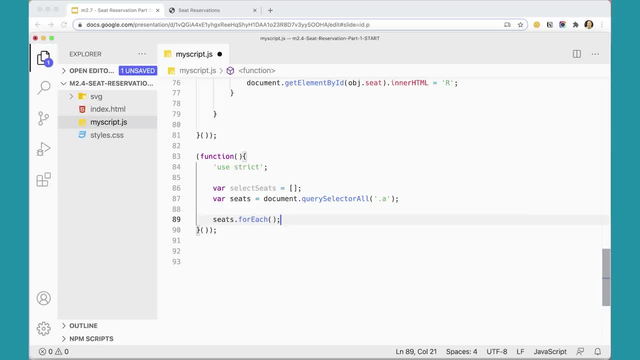 like so and the for each loop takes a function and i'm going to pass into this function seat, so each seat is going to do something in this, for it's going to do something to each seat in this for each loop, and that seat is going to get. 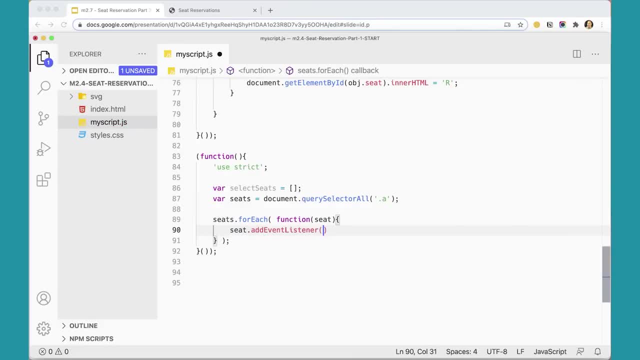 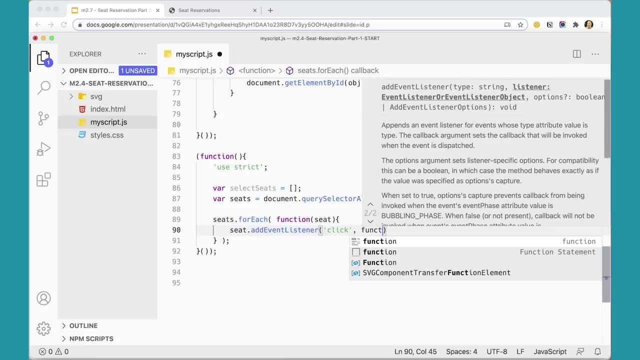 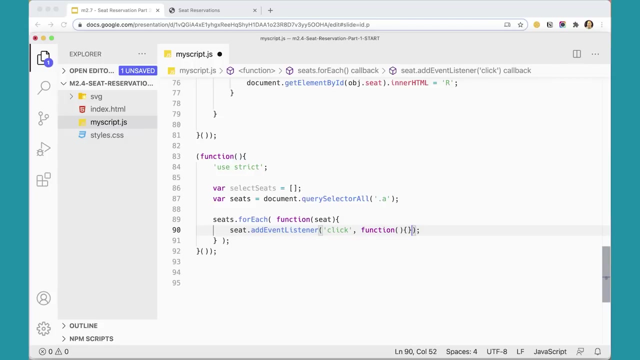 add an event listener. add event listener. and we're going to look for a click. so, And when the click happens, we're going to run a function that runs here like so, And in this function, what is that function going to do? We're going to do a couple of things. 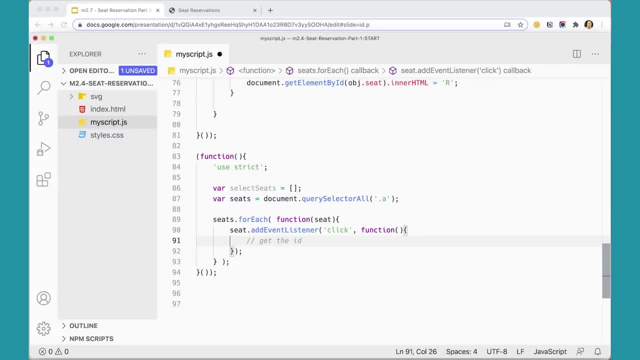 First of all, we need to get the ID of the seat that was clicked. We need to get the ID of the seat and then we need to run a function that adds it to the array. So that function is going to be down here. 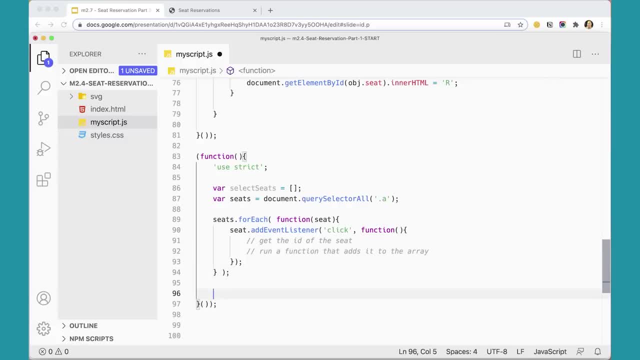 So, after the foreach loop here, which ends down here, so that's where the foreach ends- we're going to make a function that runs here. So we're going to make a function that runs here. So we're going to make a function called seatSelectionProcess. 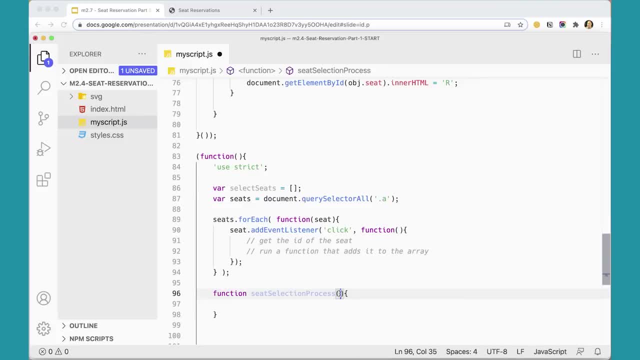 And that's going to get passed in some sort of seat, ID or something. It's going to get passed in some sort of seat which is then going to, we're going to use to then add the array. add that seat to the array. 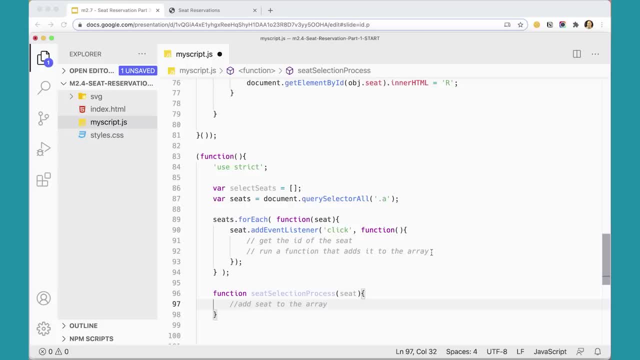 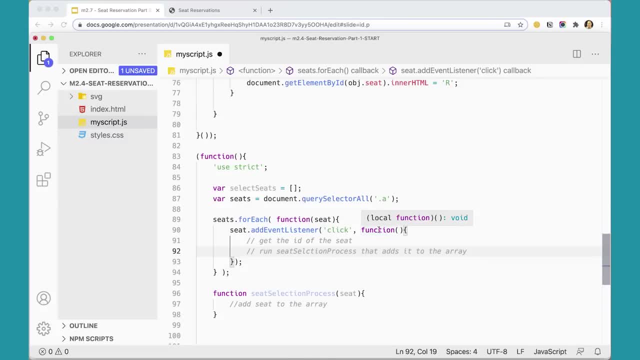 These could be good places to put in arrow functions- Both of these could be, So you could, if you wanted, to come over here and add the arrow function like that and get rid of the word function, And in this case, because seat is just one. 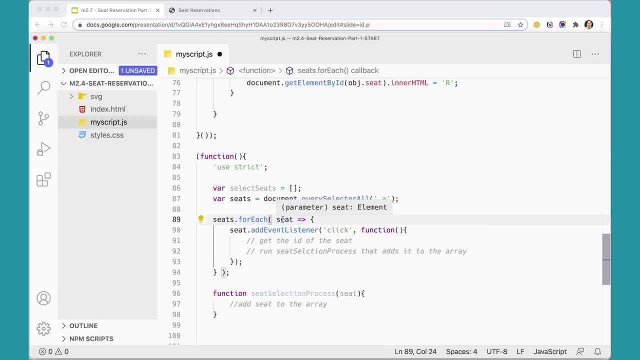 one parameter. we can get rid of the parentheses down here. We could make this an arrow function and get rid of the word function here, but we need to leave the parentheses because we don't. we're not passing in a parameter, So we need to leave the parentheses there. 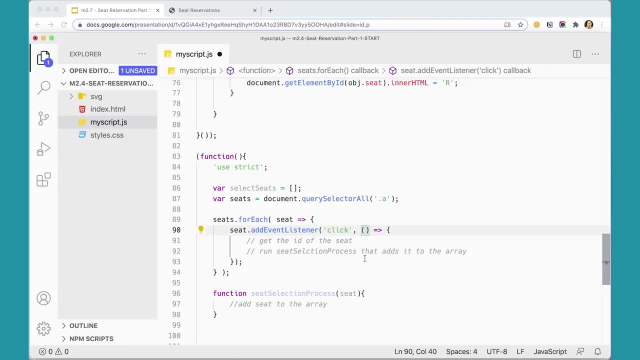 You could do it that way if you wanted to. I'm going to leave it with the functions, just because I think it's a little bit more explicit, but since we've been talking about arrow functions in this lesson, um, you could do it. 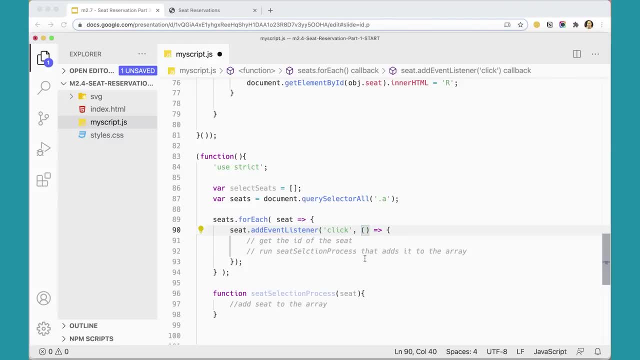 That way you can come back afterwards and just refactor down and get rid of the functions and put in the arrow functions then, which I think sometimes helps to do it that way, And I'm just going to back up here and go back to that version. 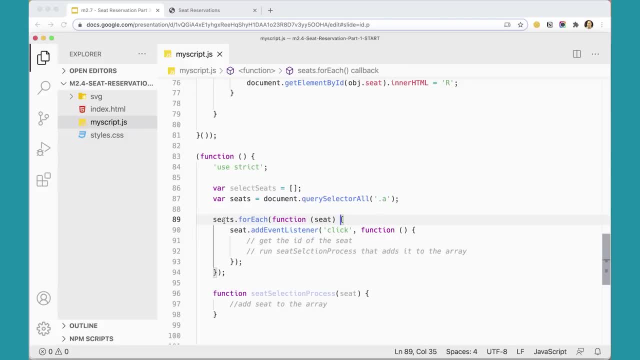 There we go. So now we have, um, a loop that's going to loop through any, all of the all of the seats with the anchor tags on them. Um, not with the anchor tags, but with the class of A on them. 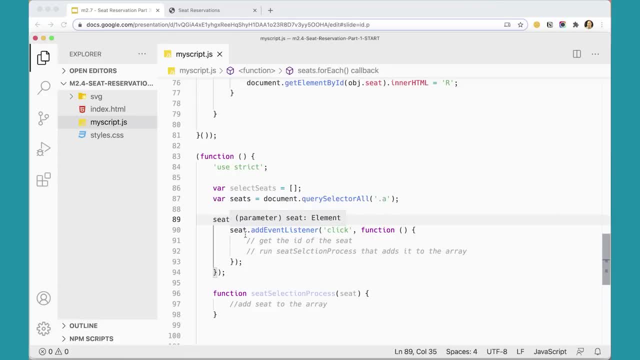 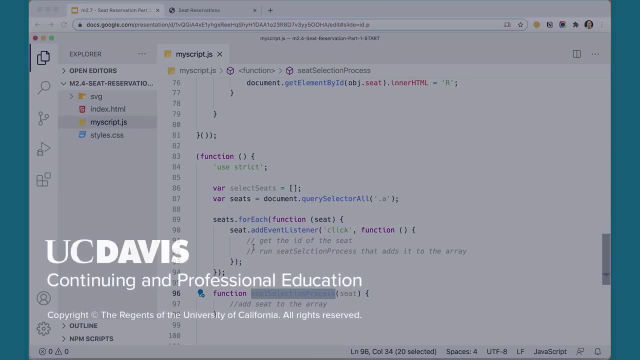 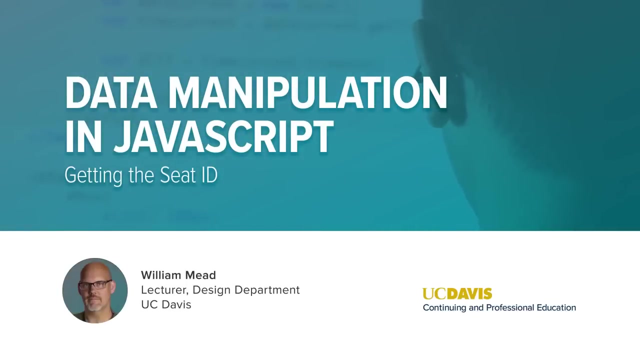 And it's going to. it's going to add an event listener to all of them. that's looking for a click And when that click happens, we're going to run this seat selection process down here. The next challenge is to see. well, okay, 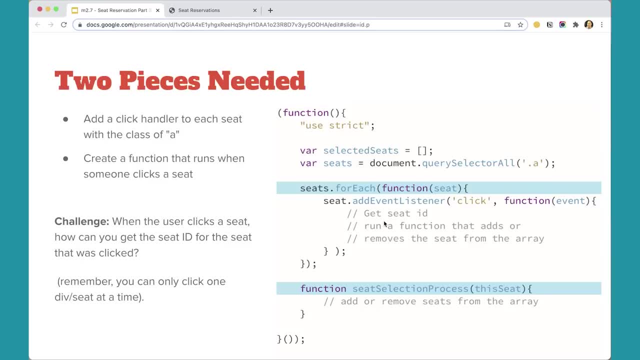 When the user clicks on a seat and you can only click on one seat at a time, how can you get the ID for that seat? And again, one way of dealing with this is to play around with JavaScript. just sort of play around with it and see what you get. 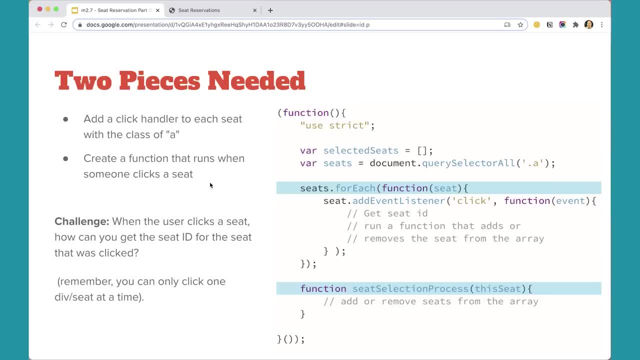 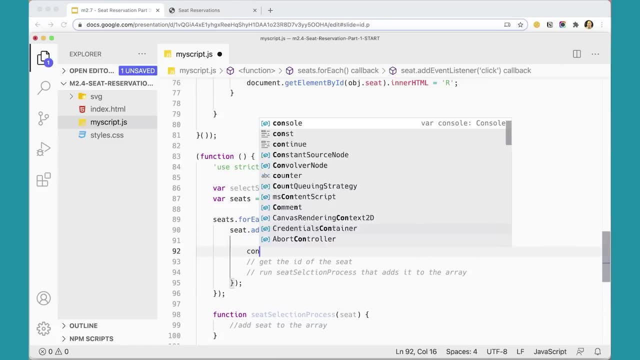 What is actually in this variable seat. Let's find out what's in that variable, If we come over here and just put in here console dot log seat and then come over and refresh our page over here When I click on one of these. 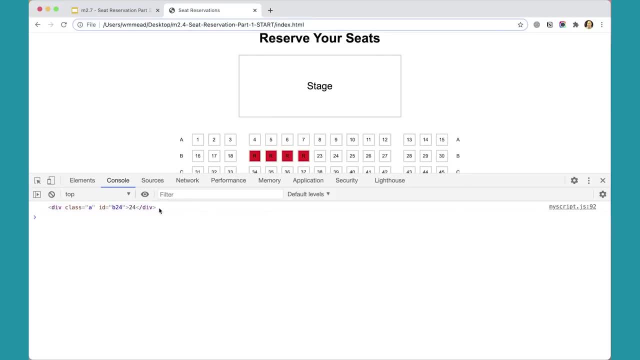 I get this. I get the entire div. when I click on one of these seats, I click on this one, I get that one, but you can see the ID is embedded in there, but I'm getting the entire div. Well, we know that ID is a property of this element. 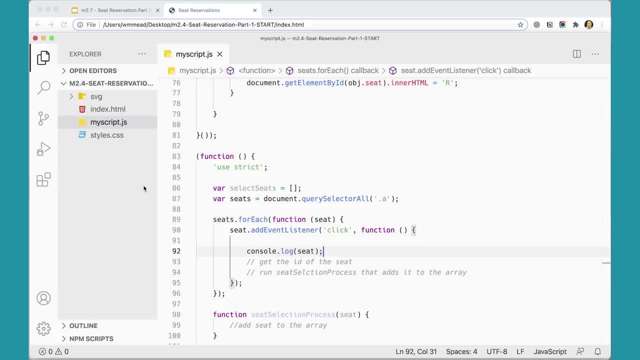 this div element. So what if I just do seat dot ID- And you may not have thought of that, because it's not- everything is a property, but in this case the IDs we knew were properties. We've seen that before. 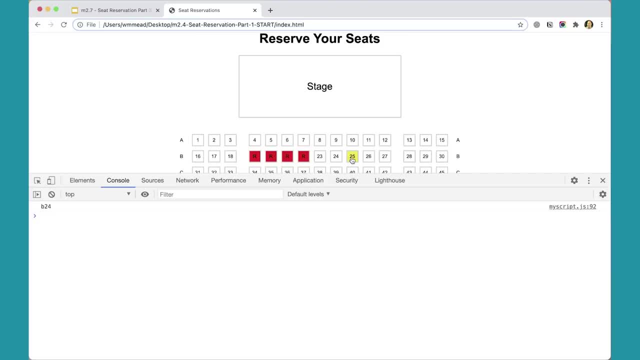 So now, if I try this and I click this, I get B 24 or B 25 or B 26.. So I can get those IDs every time I click on one of these. So I'm part of the way there. I now have the ID. 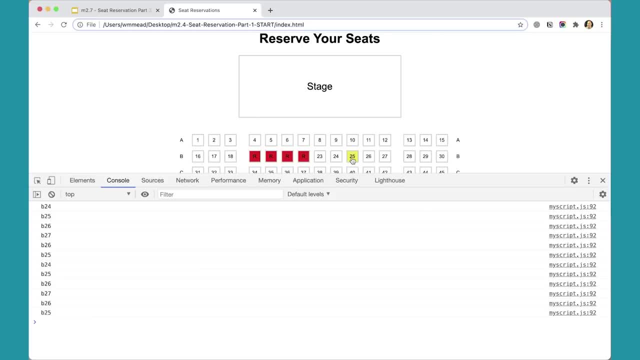 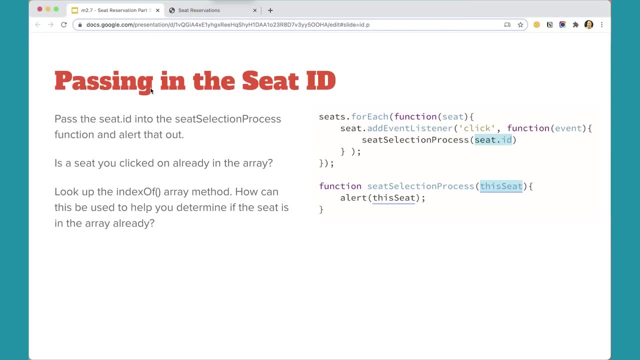 Now I just need to add it to the array or, if it's in the array, take it. Okay, it out of the array. so when i run my seat selection process here inside my event listener, i just need to pass in seatid and that will be the id of the seat that was clicked. 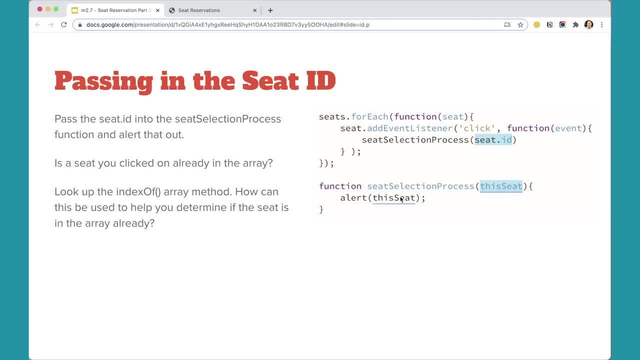 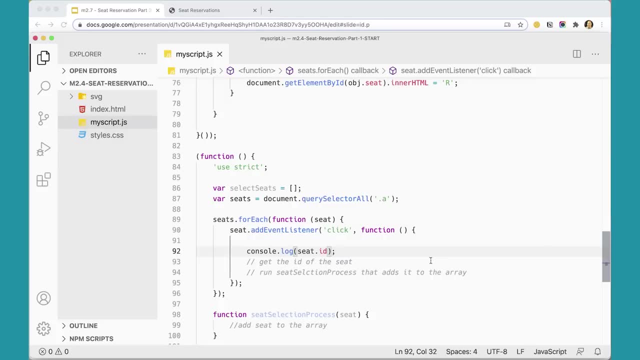 and i can test this by even just doing an alert down here in this function. so let's try that really quickly. if i come back here and run this function, i'm going to take out this console log, because i don't really need that anymore, or in fact i'm going to just delete all this stuff. 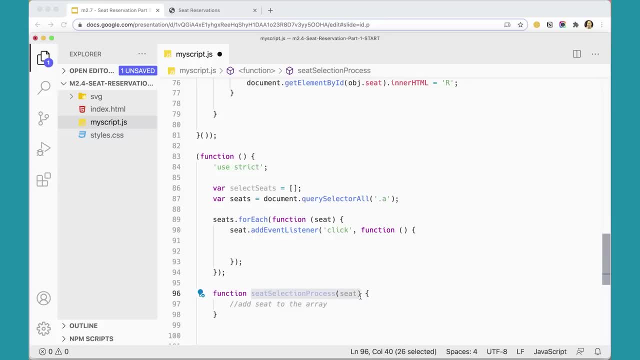 and in here i'm going to run seat selection process and here i'm going to put in seat dot id. that will pass that in as a as an argument here in place of seat. and to be really clear, i had put in here um this seat because it's a very specific seat. it's the seat that was clicked in. 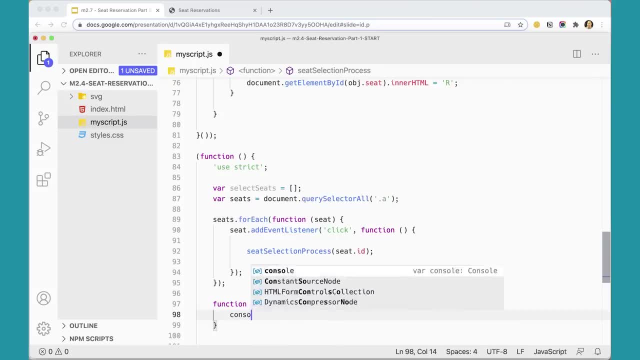 clicked on and so down here i could do consolelog this seat to see for sure consolelog. or i could do alert and put an alert. so let's do alert so i can see for sure that this function is running and it's getting the particular seat that was passed in. so let's just test that really quickly. 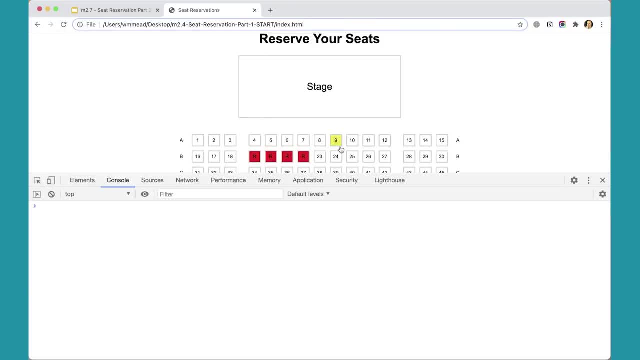 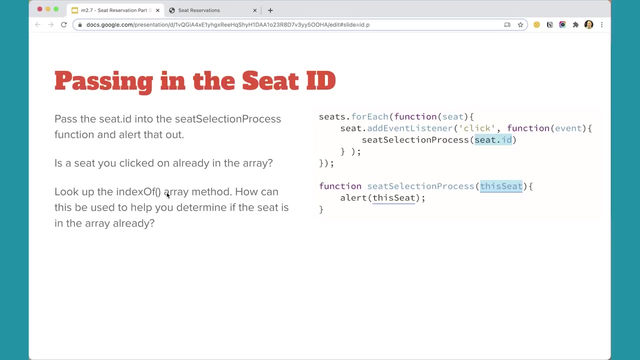 if i come over here and refresh this now, when i click on a seat, i get an alert that says b24, because it's running that function and putting that in there. okay, the next challenge for you to do is to figure out. okay, how do i know if i've previously clicked on the seat? 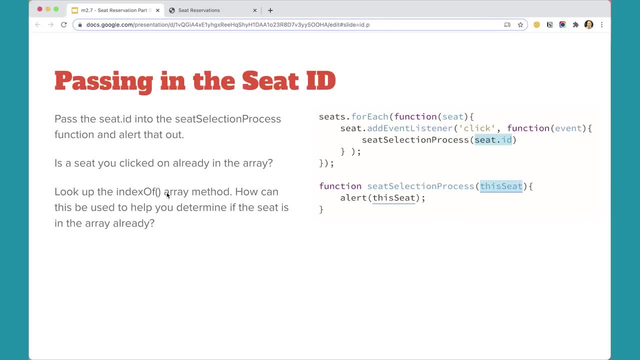 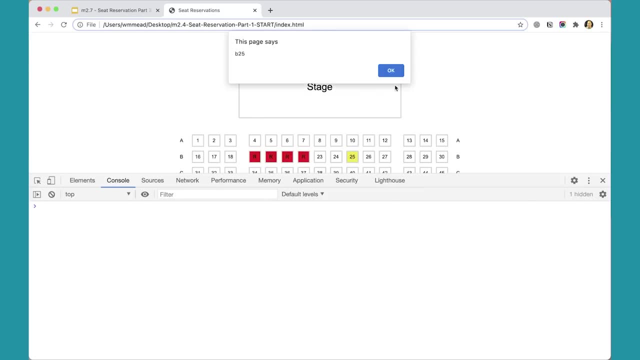 we know that we can add stuff to the array using push, but how do we check in the array? i'm going to do that- something's already in there- because i want to make it so that if i click on seat 25, that one gets added to the array. seat 26 gets added to the array, but if somebody clicks on seat 25 again, 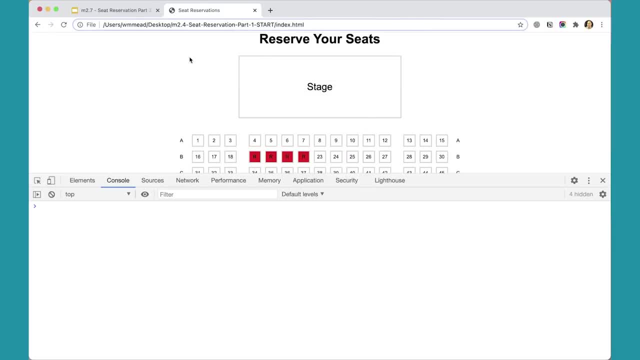 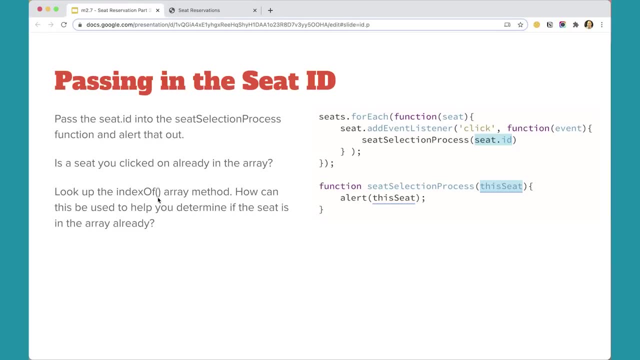 it gets taken out of the array. and if you look up the array of the array method index of on the mdn, it can give you some information about how how we could possibly make that work so we can take things in and put things into the array and take them out of the array based on whether or not they're already in the array. 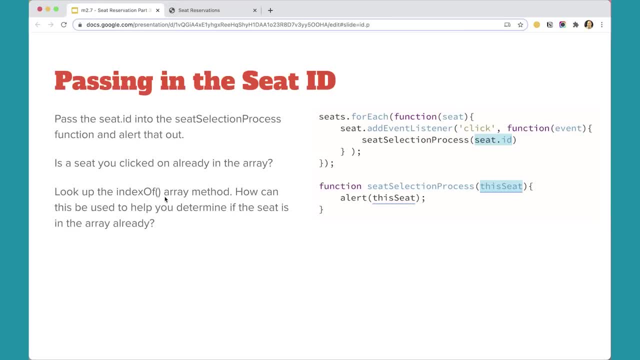 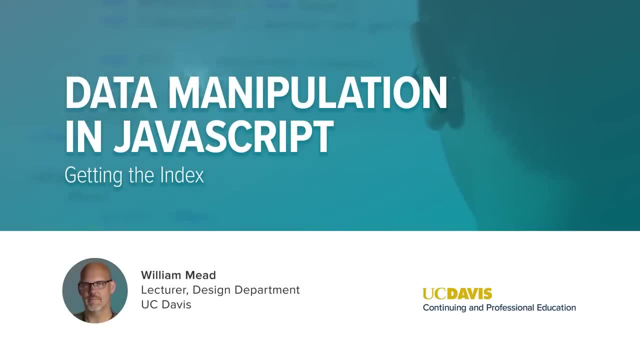 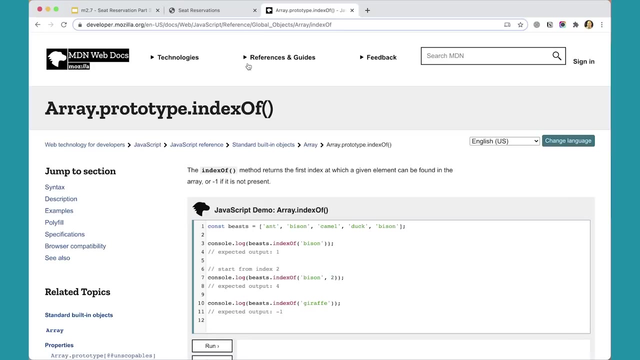 so take a look at that and see what you can figure out, and then we'll look at it in the next video together. and if we go over and actually look this up on the mozilla developer network, you can scroll down here and sort of get some examples of how it works. so if we have a simple 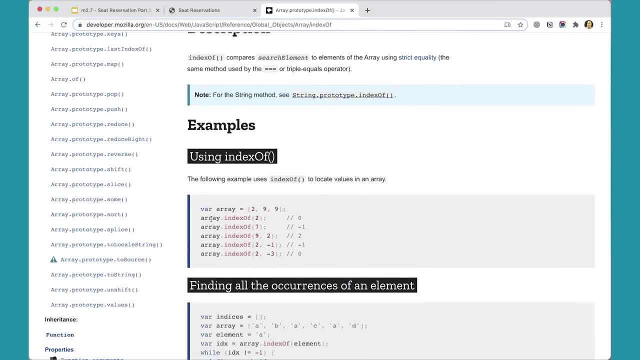 array with two and a nine and nine in it. if i do index of two, that'll, that's that element. it'll tell me it's at index zero. if i do index of seven, there's no seven in the array, so it'll give me a minus one, and you can continue to look through some of the examples on this page and mess around. 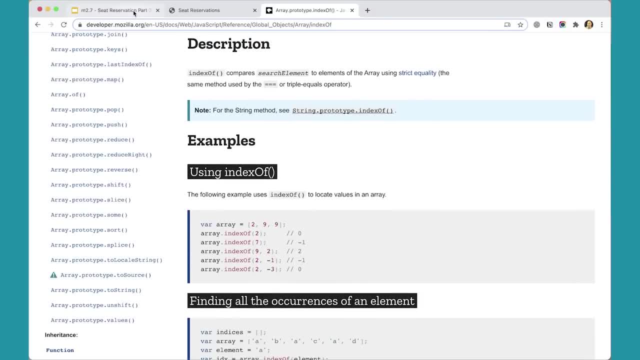 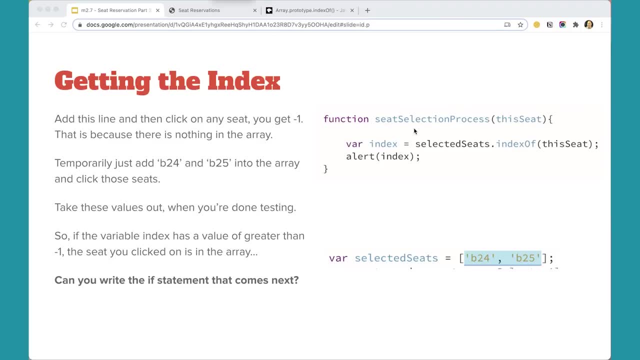 with index up to try to get this to work. but over here, if we just play around with this a little bit, suppose in our seat selection process function here we make a variable called index and we go and say seat- selected seats- index of this seat and alert that out, we should get a minus one because our selected seats array is still. 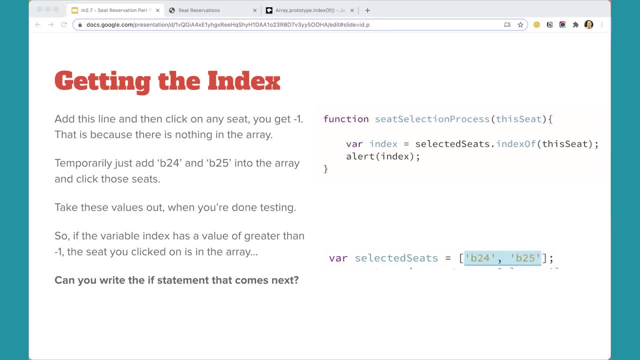 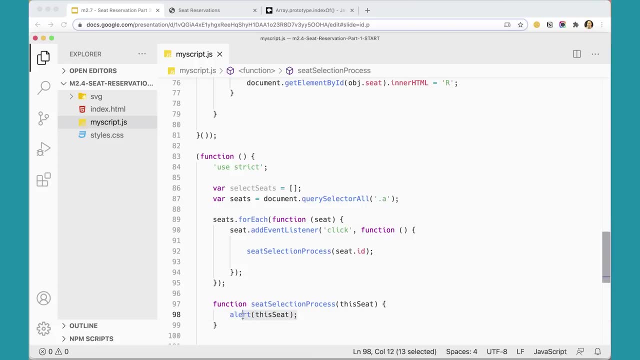 empty. so let's see what happens if we do that and see that that's actually working the way we think it's going to work. so down here, if i change this to var index, equal seat, selected, selected seats, dot. index of, and i'm going to pass in this seat, which we know is the id, this seat, 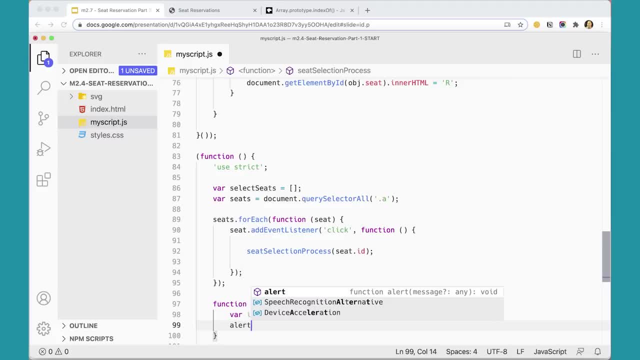 and then i'm just going to alert out alert index just to see what i get there, and i should, because that array up here is still empty. the window is still empty. no matter what i click on, that should come back with a minus one. so let's just test that much and see what we get if we come over here and refresh this and then 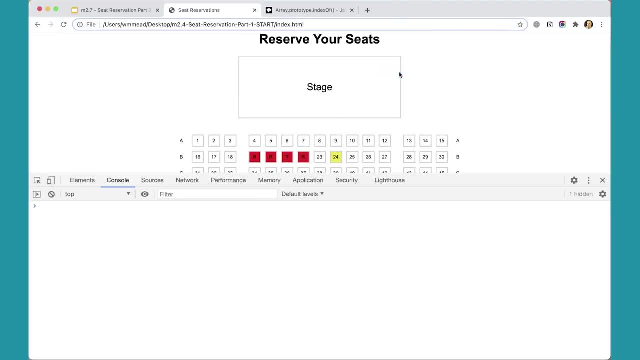 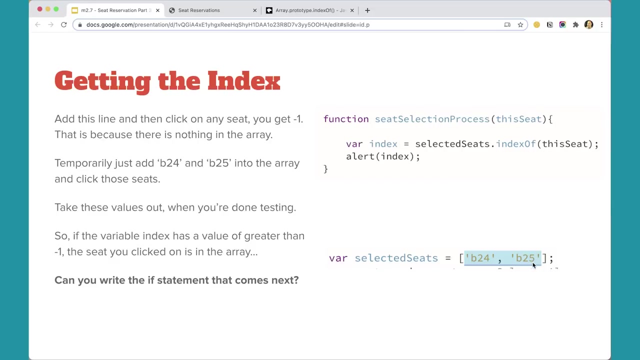 click on the c, i get a minus one. if i click on a different c, i get a minus one. if i click on a seat over here, i get minus one because nothing is in the array. okay, great. so what if, just for a temporary moment, we just add a couple seats in the array? what do we get then? if i add b28? 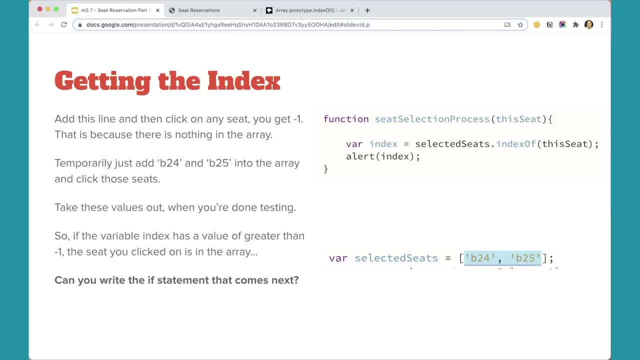 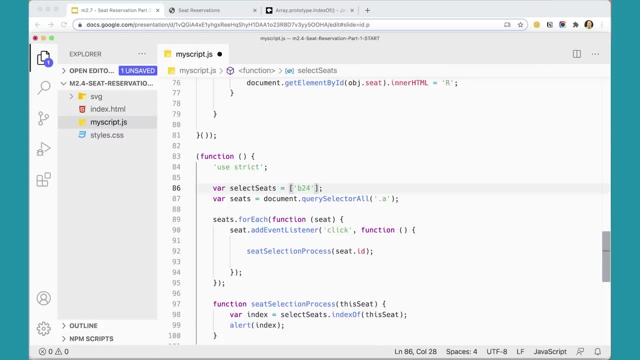 B24 and B25 into that array, just temporarily, just to experiment and see what happens. So up here I'm going to just put B24 and comma quote: B25.. So now if I come back and click on here and if I click on something that's not B24 or 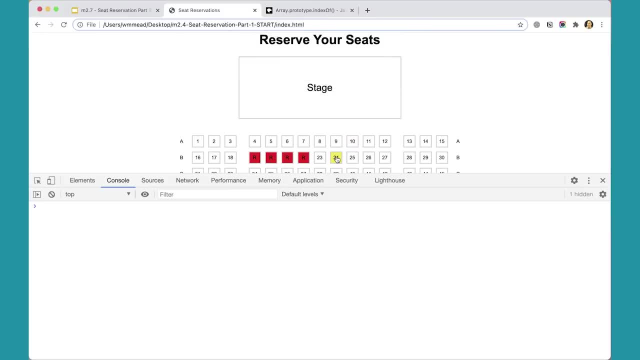 B25, I still get a minus one. But if I click on B24, I get a zero. If I click on B25, I get a one. So essentially what we've learned here is that if I click on a seat that's in the array. 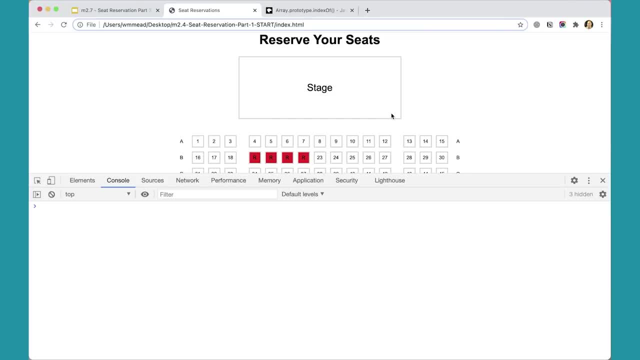 I get a number larger than minus one. If I click on a seat that's not in the array, I get a minus one. So that should help us put together an if statement that says: if the index of is minus one, then it's not in the array and it should be added. 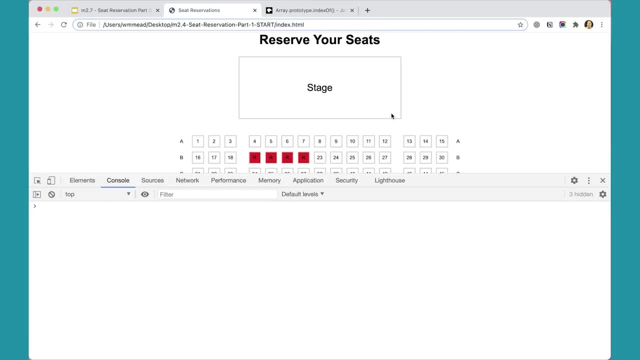 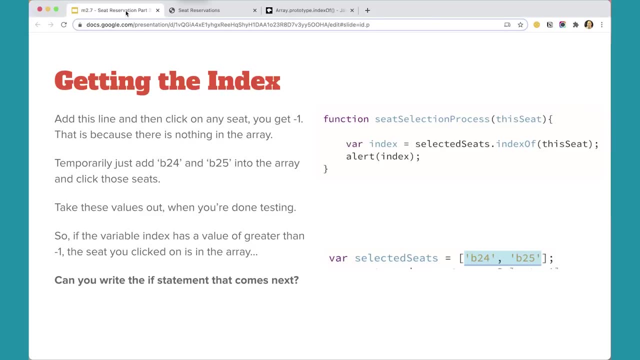 Otherwise it must be in the array and we want to take it out. Correct: Your little micro challenge here is to write that if statement, not fill out all the contents of the if statement. but what does the if statement itself look like? 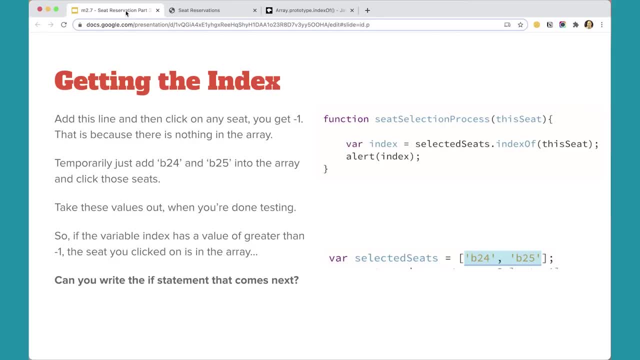 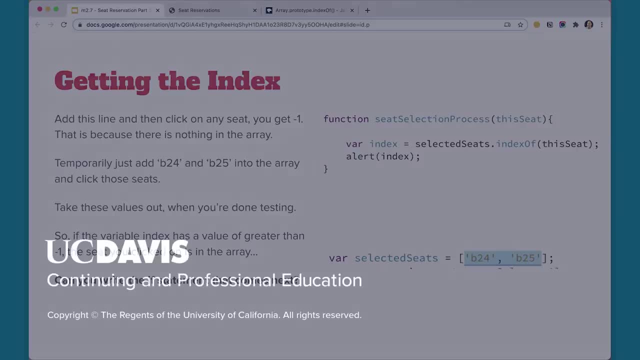 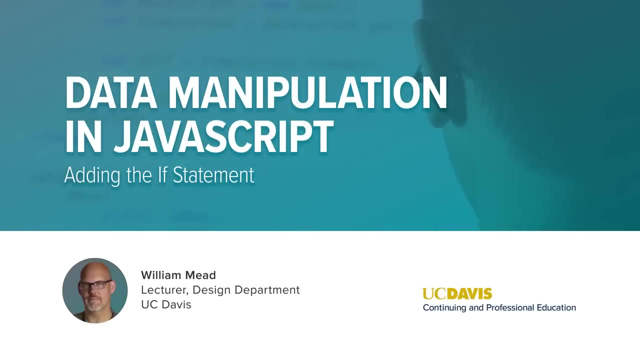 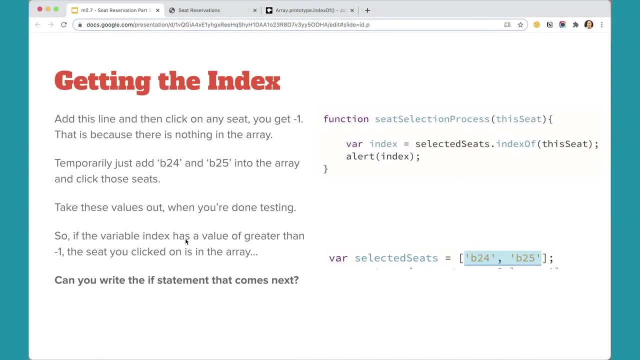 How do we write that much? Just get the if and the if statement in there and see what that looks like, And we'll look at that. look at the answer to that in the next video. Your challenge was to write the if statement that we would need to use to determine if. 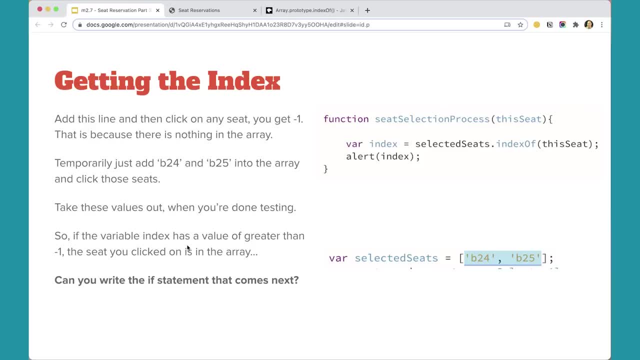 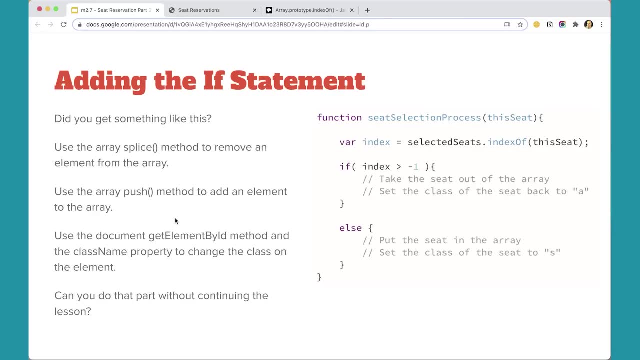 an element that's clicked on is in the array or not, And so let's see what you came up with. Did you come up with something like this? Hopefully you did So. if so, I have a variable here: var index equals seats, selected seats- index of this. 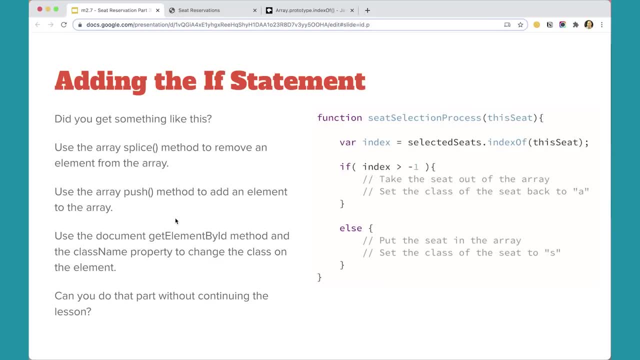 seat, And if index is greater than minus one, then it's in the array and we can take it out. Otherwise it's not in the array and we need to add it. So let's go ahead and add that over to our code over here. 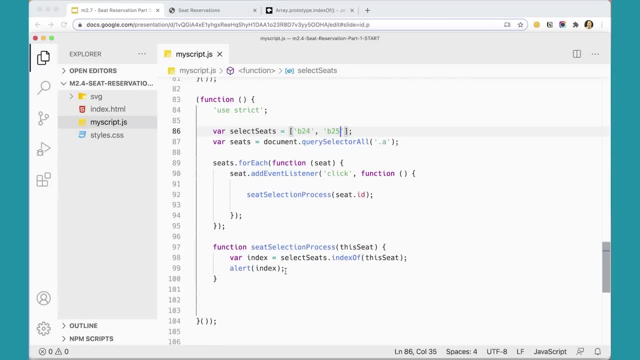 We already have this variable here And really all we need to do is take that out and add an if statement. If index is greater than minus one, Then it must be in the array. Must be in the array. Take it out and set the class back to a. 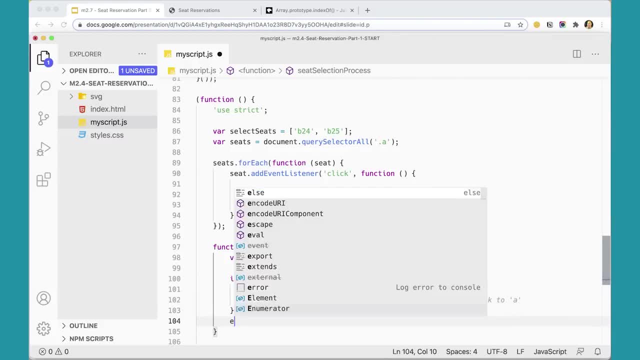 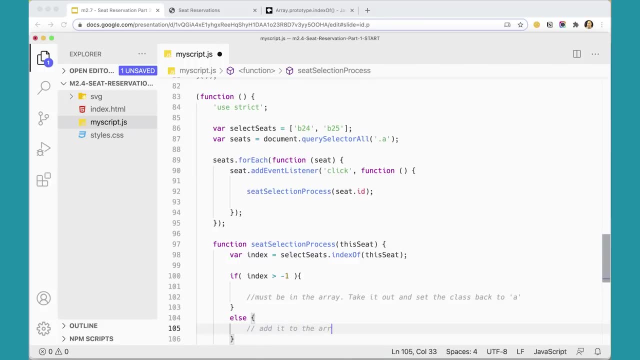 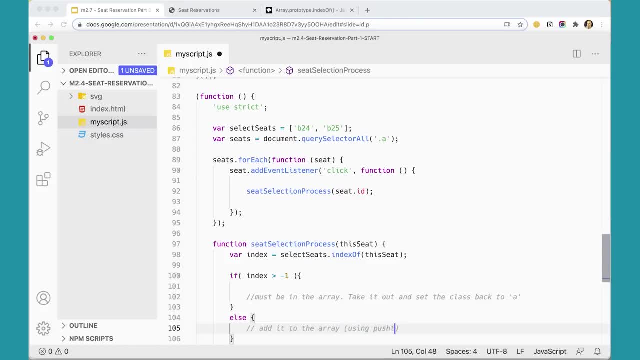 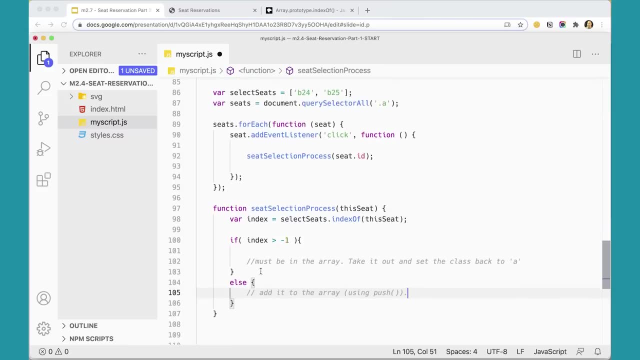 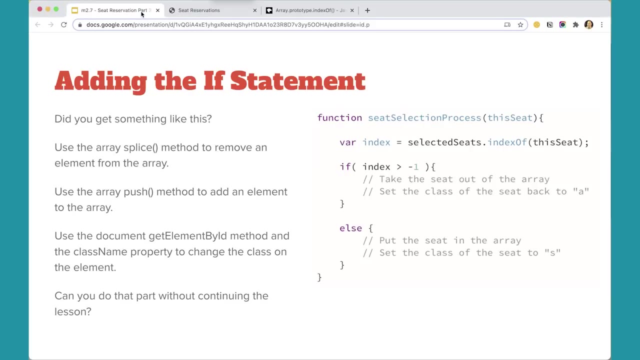 If, If, If, Using push. We'll use push to do that, right? Okay, So there we go. We've got that. We've got that far. Your next micro challenge is to fill out these if else statements. So if the seat's in the array, we've determined that it is because it will return a minus one. 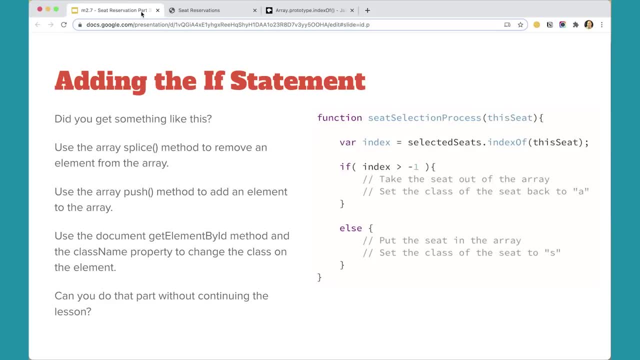 index will have a minus one. so if it's, if it's not minus one, we want to take it out of the array. and because index has in it the value, which is the specific number in the array that it is, uh, we, we know what. we know what it's going to be in the array, so we can take it out. um. 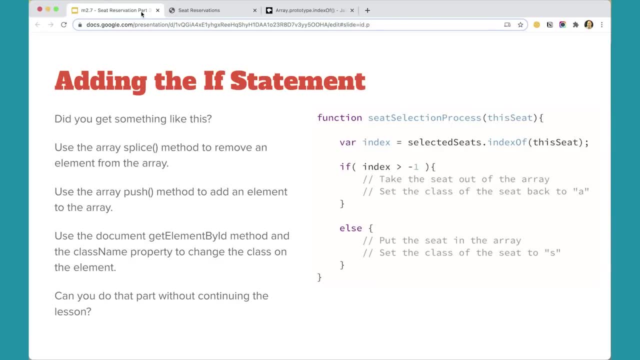 otherwise we want to put it into the array and if we're taking it out of the array we want to set the class of that seat back to a and um. if we're putting it into the array, we want to set the class in the seat to s for saved. it will get turned to reserved when we actually 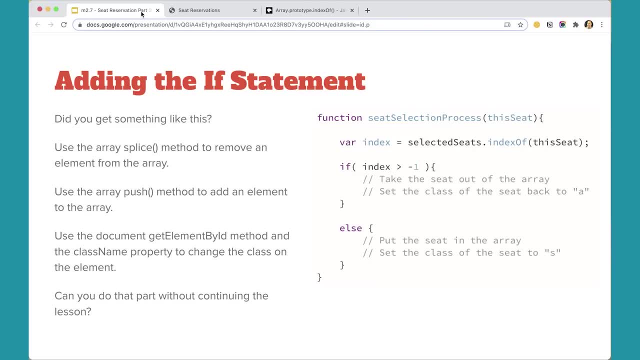 reserve the seats in the in the next and in a later part um of the of this lesson, but um, for right now we just want to set it to saved, so, and we have already have some styles in the style sheet that will take care of that. but uh see, if you 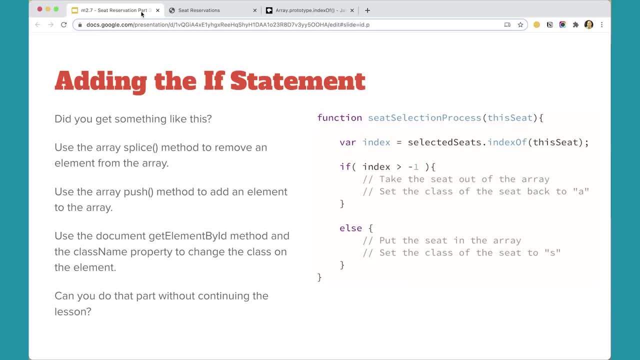 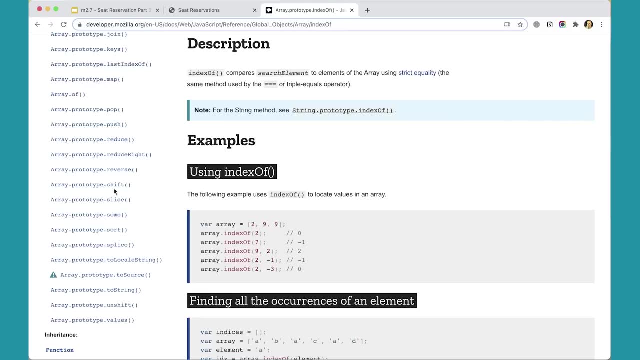 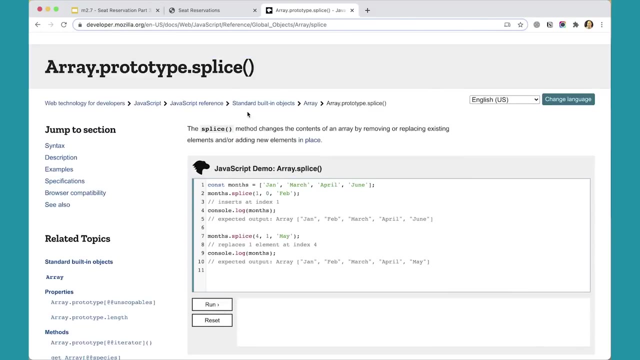 can do this part on your own and to take it out of the array, look into using the splice method. so if we go back over here and click on splice, you can actually look through this page to see how you might use the splice method to take that element out of the array. so let's see. 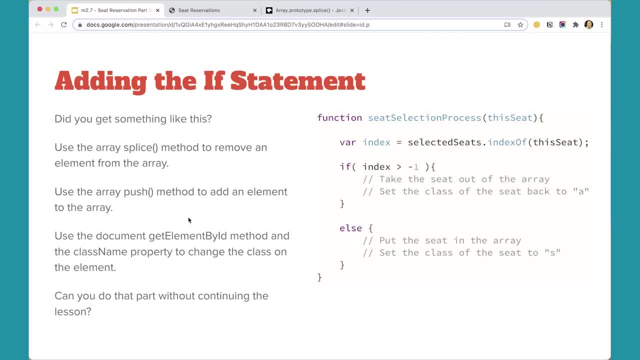 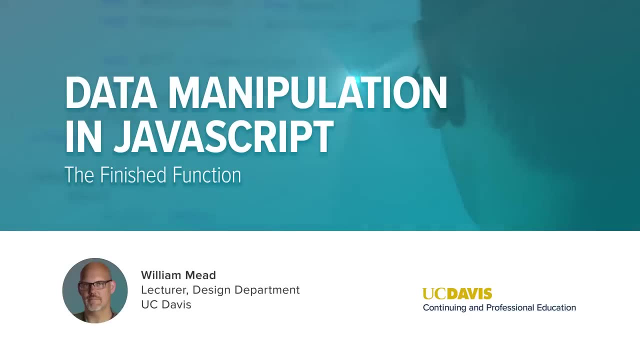 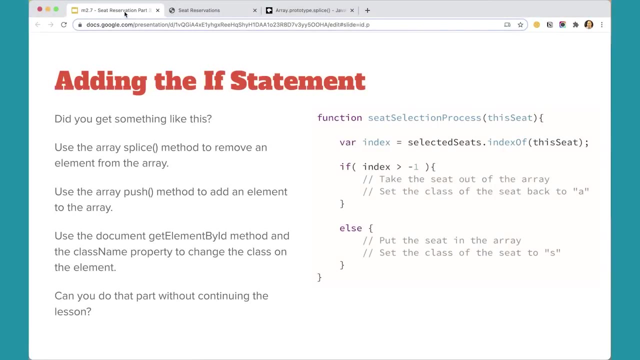 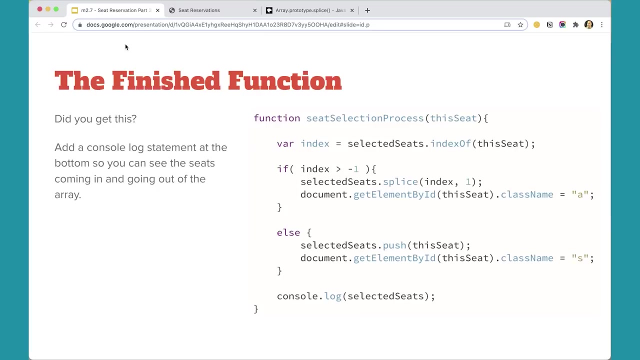 if you can do that on your own, and then in the next video we'll look at my solution for that. how did you do with the micro challenge? were you able to complete it? hopefully you got something like this: we're going to use the splice method and we're going to pass an index because index. 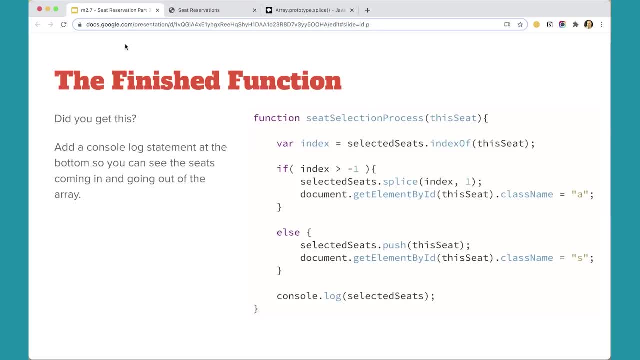 will tell us which element we want to remove, and splice takes two parameters, and the second parameter will be: how many elements do we want to actually remove? and we just want to remove the one, the one that we clicked on, so we'll put a one in there and then setting the class name. 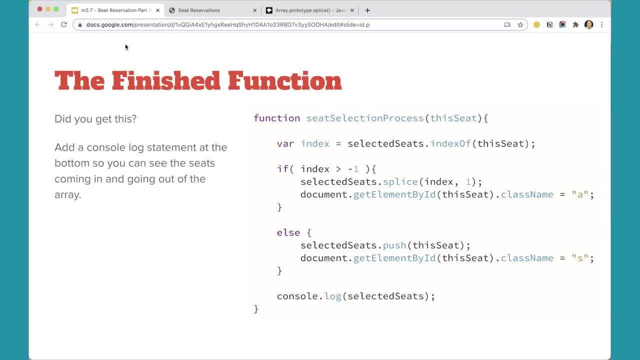 is as simple as using get element by id and using this seat- we know that that has the id for the seat- and using the class name property to set it to a. adding the seats into the array is just using the push method. we've done that before in previous lessons, so we can just push this seat into the. 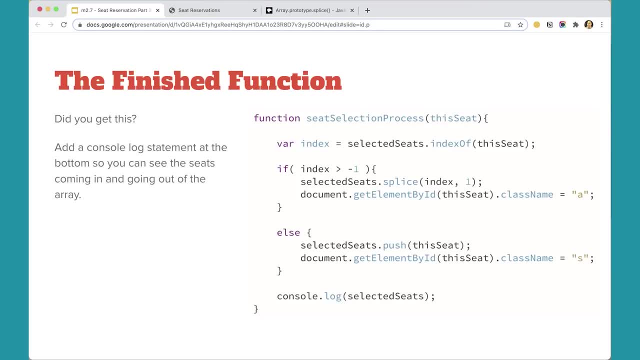 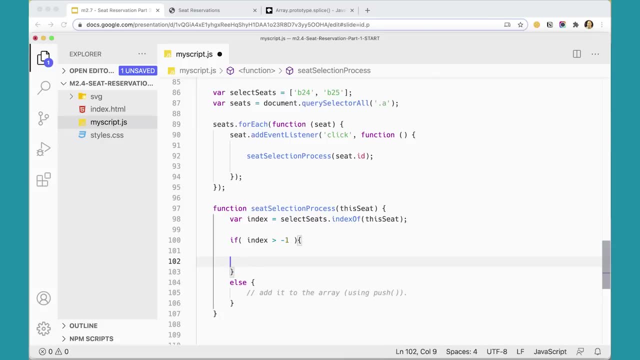 array. so let's go ahead and add this over into our code over here. so under the if i'm just going to do selected seats, dot splice, and what am i going to pass in there? i'm going to pass in index comma 1.. so that will take that element out of the array if it's in it. 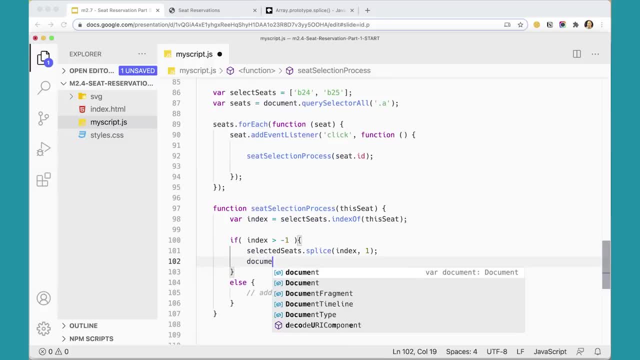 and while i'm there, i want to do document dot get element by id. this seat, which i know, is the actual id dot class name. if i'm taking it out of the array, i'm going to set it back to available and that's all i need there down here instead of. 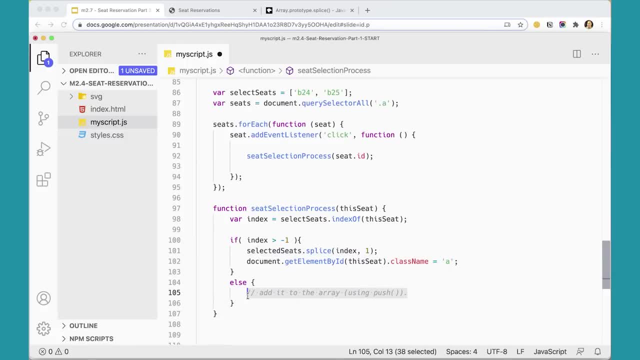 instead of removing it from the array, i'll just copy that, because that makes it a little bit easier. paste it, but instead of splice i'm going to do push this seat. i'm pushing that id into the array and then i'm going to take this line because if it's in the array, the seat is currently going to be. 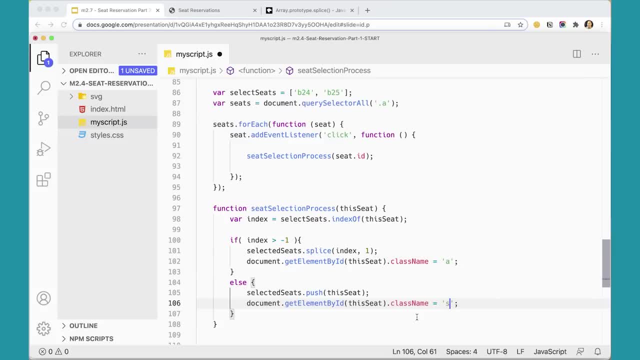 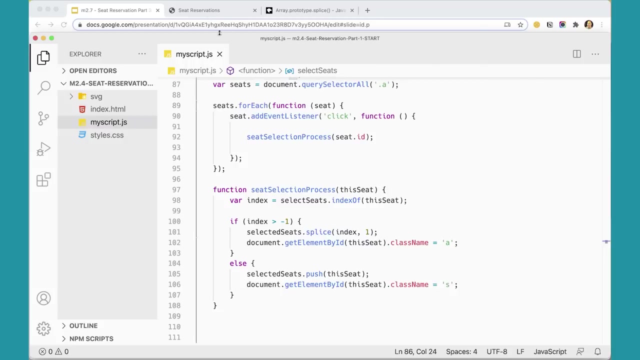 saved like so, and then up here. i just want to remove these things that i temporarily added into my selected seats array so it puts it back to empty there and let's see if that works. i think it should. if we come over here and refresh this. actually, i think we're going to have to console log. 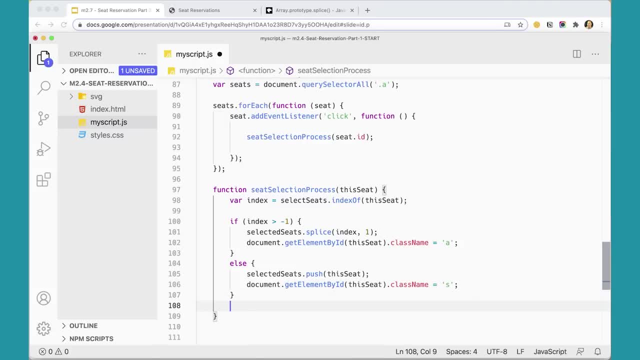 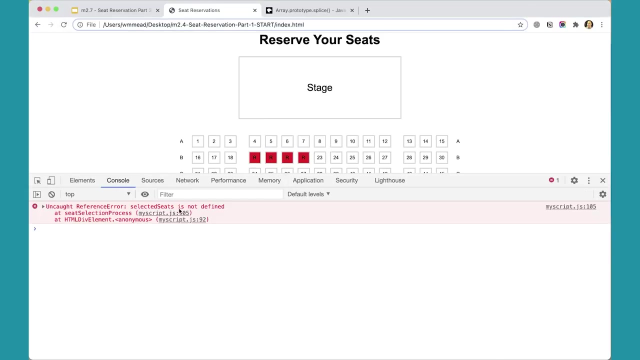 something out here that's at the bottom here. do console dot log selected seats so we can see what's going in and coming out of that array every time we click on a seat? all right, let's try this out. if i click on b24, whoops, selected seats is not defined. 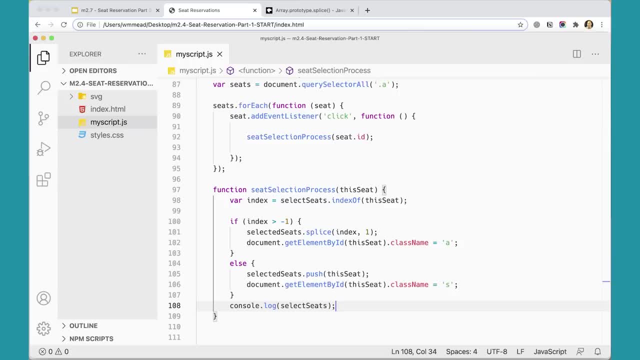 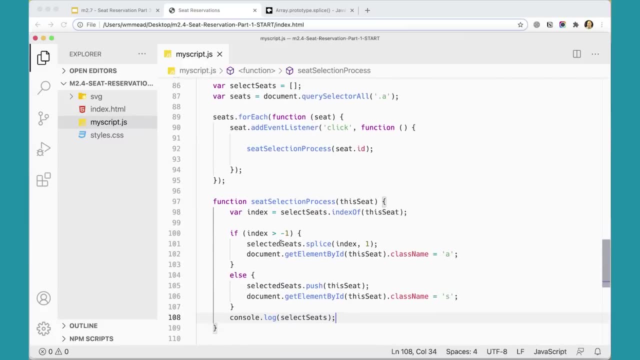 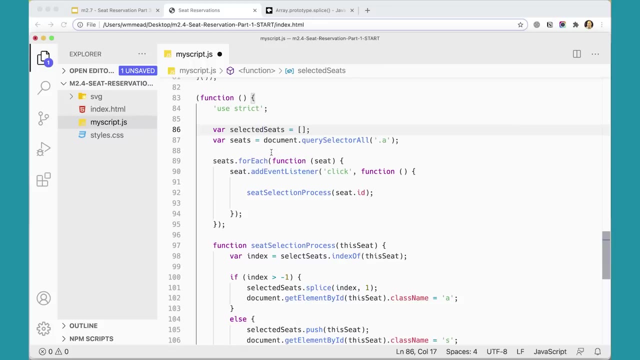 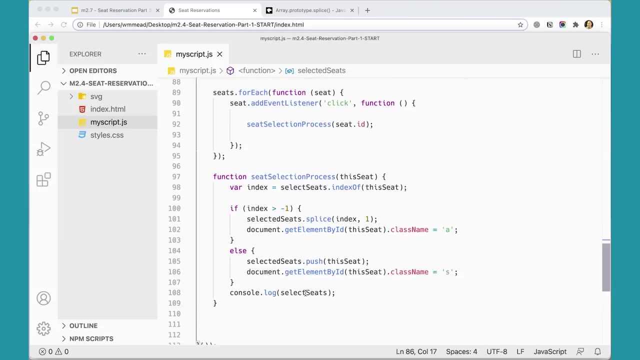 what did i do wrong there? online 105 selected select seats. i'm going to change this to selected seats because i think that's what i originally had: selected seats. there we go. that makes more sense. console logout, selected seats. okay, check it again. these mistakes happen. i make them all the time. you'll make them too. 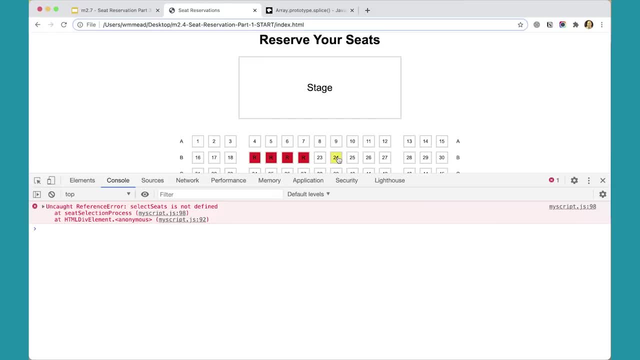 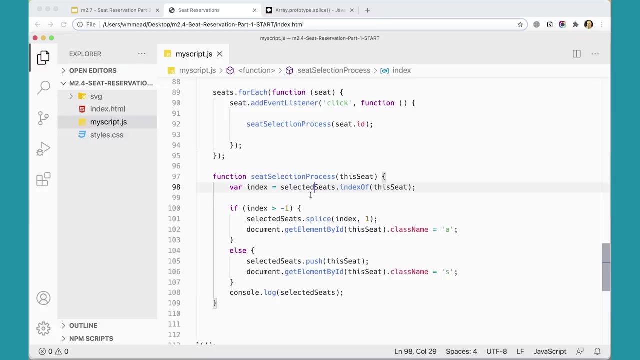 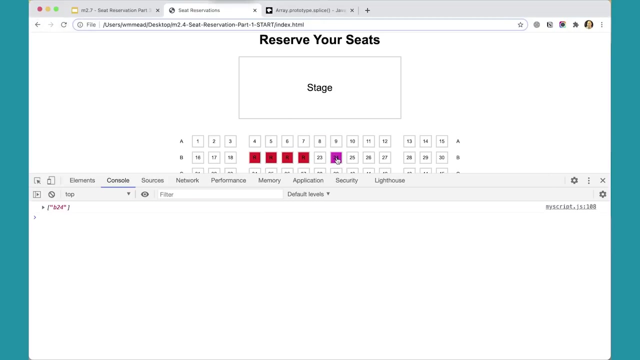 and it's. it's helpful to use that console log to figure that out. oh, i still have select seats in there. i might need somewhere. this is why it's a good idea to always copy and paste your variables there we go fix that so that one got. 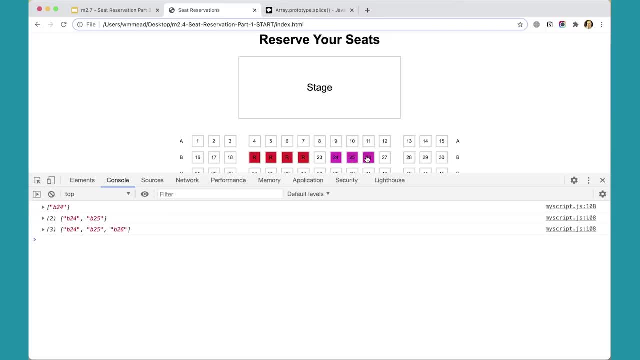 out of the way, so that one got out of the way. i can add 20 now. they're both in the array. now i've got three of them in the array and if i click on 28 again that'll come out of the array 25. the array is empty. i can put items. 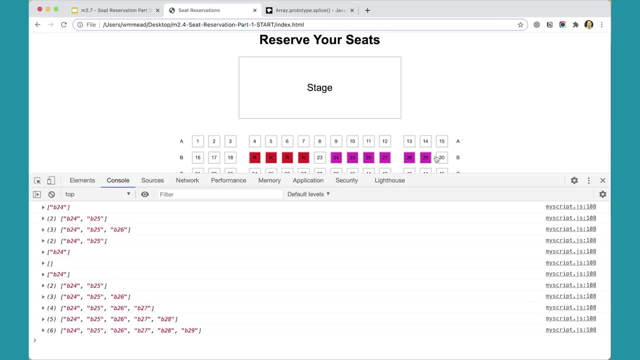 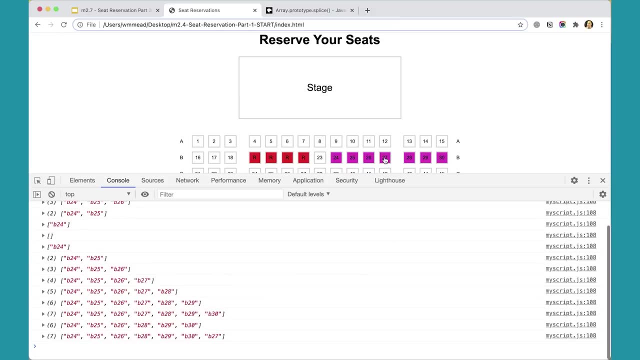 into the array. i can add more. i can take any one of these. i can pick one in the middle. it'll come out of the array if i add it again. notice, it gets added on at the end, but that's fine. we just want to know what's in the array and what's out of the array. those are the seats that i've selected. 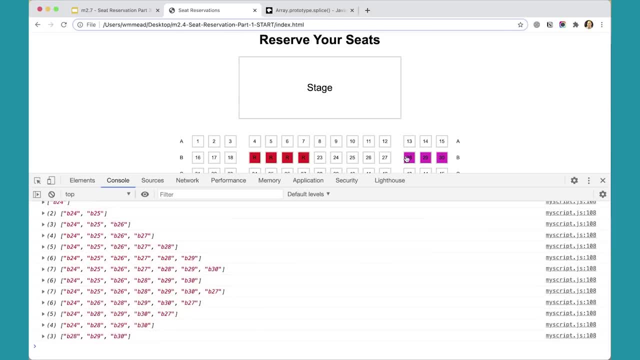 currently have selected. so this array contains the seats that i need, whatever seats that i'm currently selecting, and it's removing any seats that i select. the second time notice: i can't click on these because those don't have the event listener on them, so they don't have the uh, the. 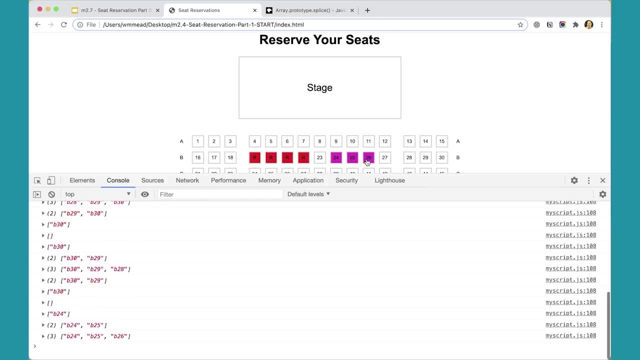 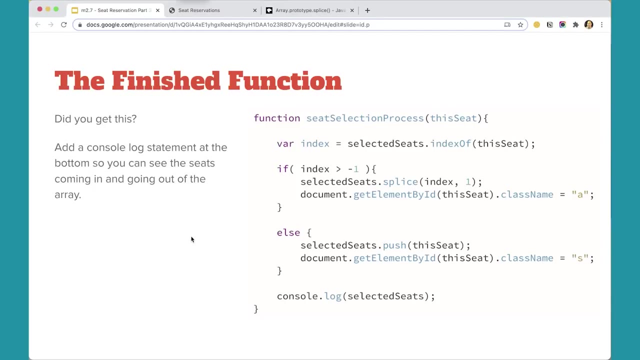 a class on them. now we will have to come back and modify this method, this function, a little bit later, but for right now, this is doing pretty much exactly what we need it to do. here is the finished function that we have in the next part of this project we will be building up. 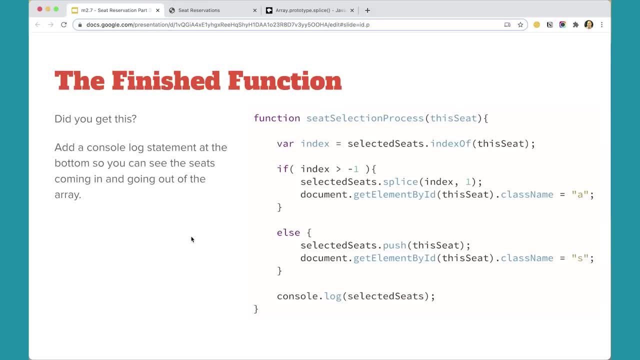 the form, the reservation form- and handling that part of the user interface. so we'll be doing that next, but this is where this function needs to be for now. we will make some minor changes to it a little bit later in the project, but this is doing exactly what we needed to do at this point. 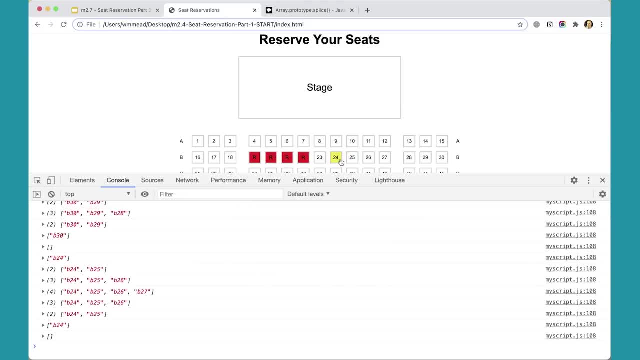 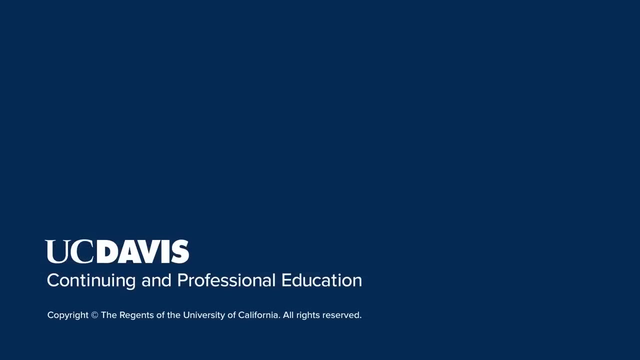 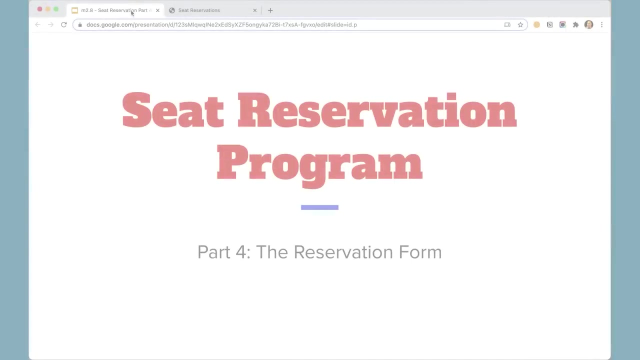 so, at this point, what we have is we have an interface that allows us to select seats and put them into an array, as well as an interface that allows us to pull from an object and show seats that have been previously reserved. okay, great seat reservation program. part four: the reservation. 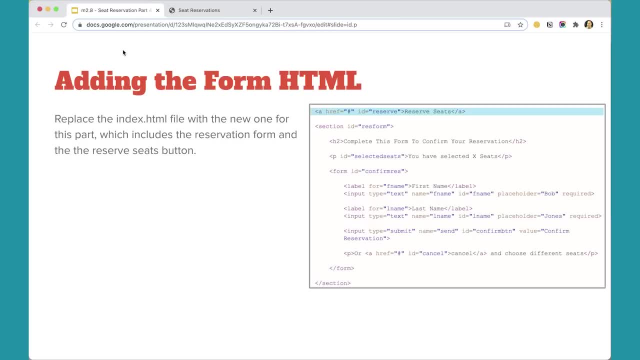 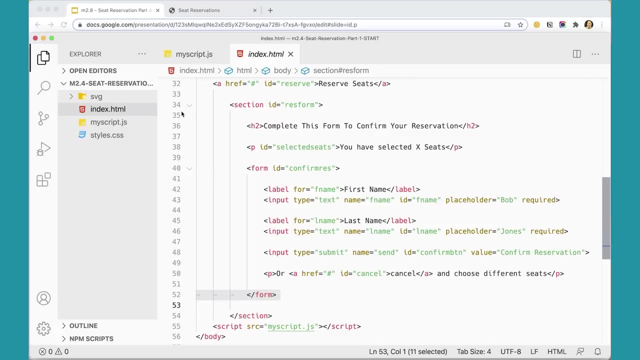 form. in this part we'll be adding a form that users can fill out to reserve their seats. and to start with, you want to replace the html file in the folder with this new version and i've already done that. it's over here in my file here and you can see in. 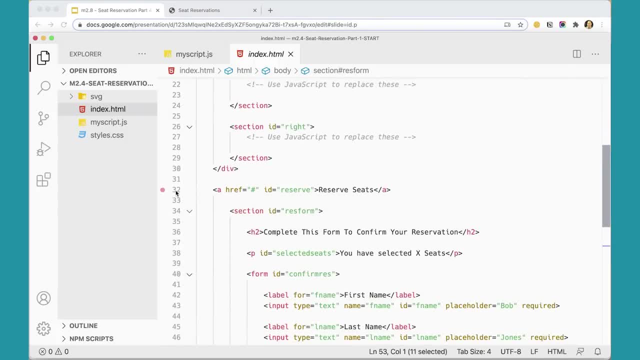 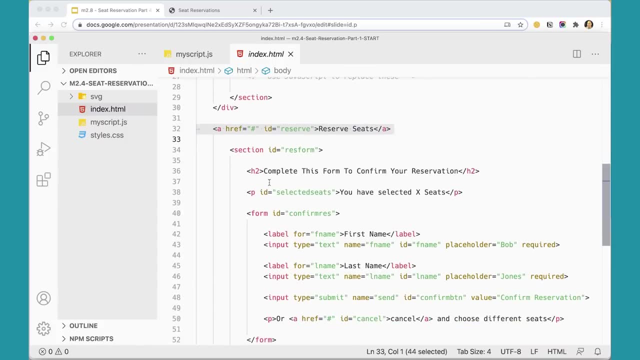 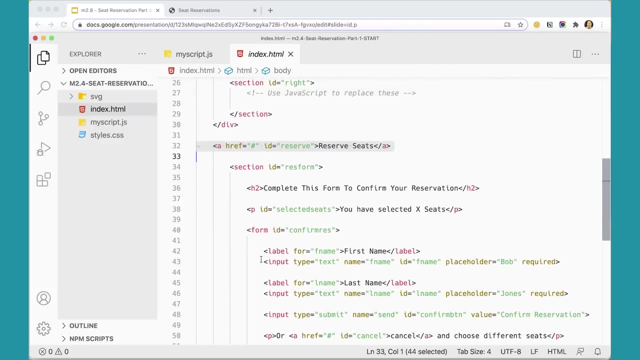 my file here, the only thing i've really added is an anchor tag for reserving the seats, and then a section which has in it a header and a paragraph and then a form, and then the section ends and that's that's it. so that's just been added in there. 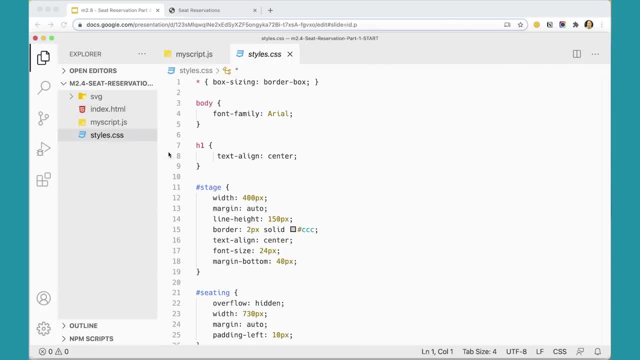 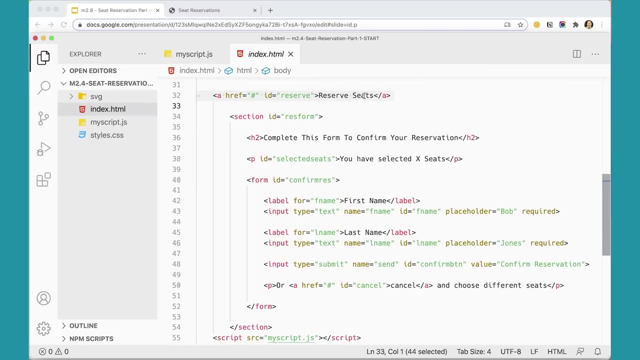 and the css for handling all of this is already over here in the css, so we don't need to really worry about styling for this stuff. i've put it in the css for us, but it is all here on the actual html now. if you wanted to type it, you could. it would just basically be this: you're just adding: 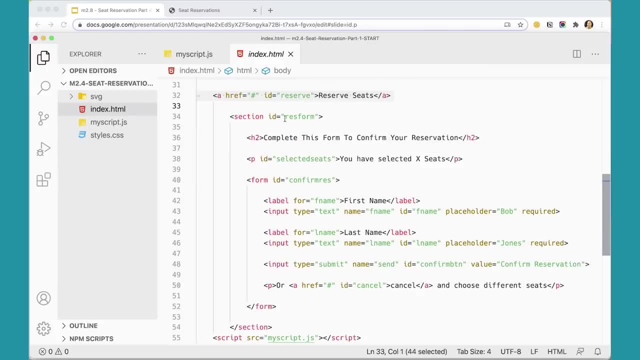 an anchor tag with an id set to reserve form, a section with the id, res form with an h2 and a paragraph with selected seats. you'll see why we're putting ids on all of these things in a few minutes. and then the form itself, which has an actual id on that one, and then we've got. 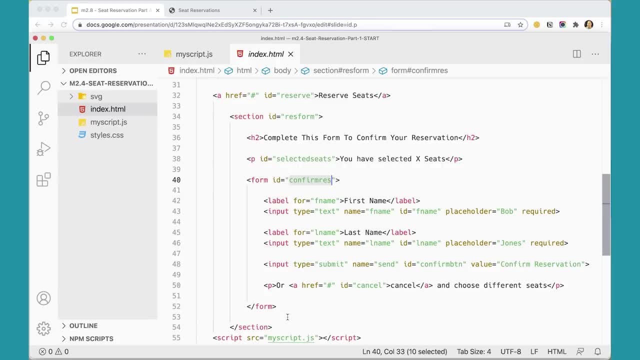 some labels and inputs so you can type this out, or you can just add the new html file that has all of this in here and replace the html file that was there before. the rest of it is the same. okay, great. it's important to note that this part of this project i'm using is the ledger to predict if this is the next level that major referee can be91. 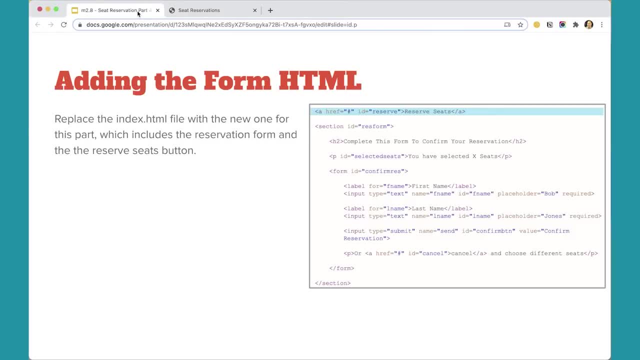 it's important to note that this part of this change, this part of this project, is probably the hardest part of this project. And it's not hard because the JavaScript is hard. It's hard because you have to really think about how users can mess up. 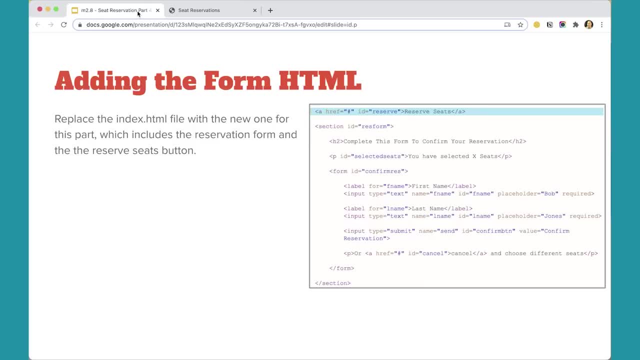 how they can screw up in the process of doing this, And there are a number of ways, even with this very simple process, that users can screw things up. So you have to think about all those things and catch them and handle all the potential errors, And that makes this part a little bit more. 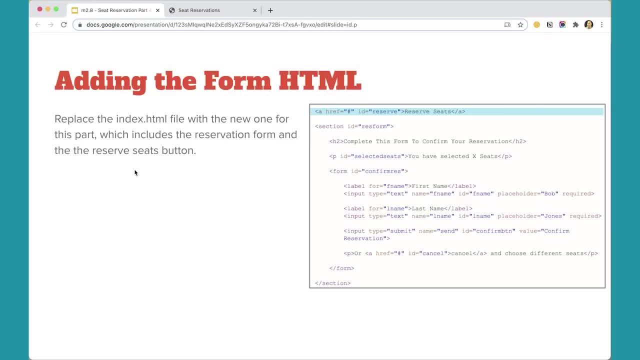 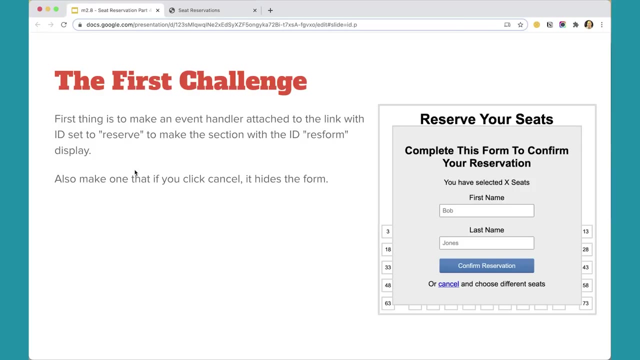 challenging in terms of the way you have to think about the programming and what's going to actually happen in the state of the application as users complete their process. Okay, so let's take a look at what we need to do next. The first thing we need to do is make an 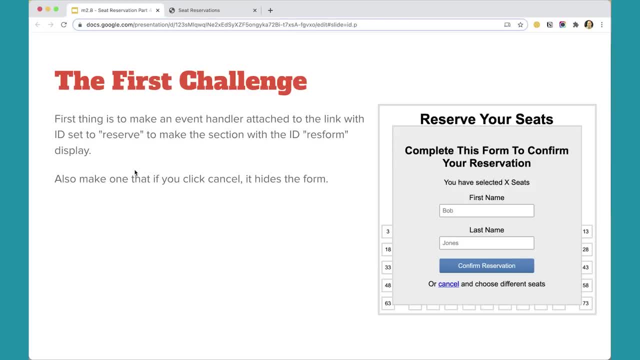 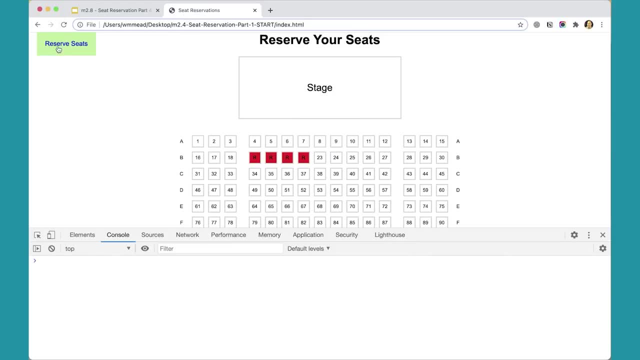 event handler. that's attached to the link. So when you click that link so over here, I've added that stuff to the page And if I come over here and refresh, I now have a reserve seats button over here. So when I click, 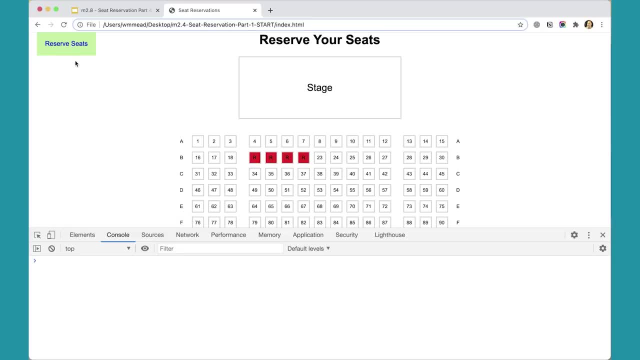 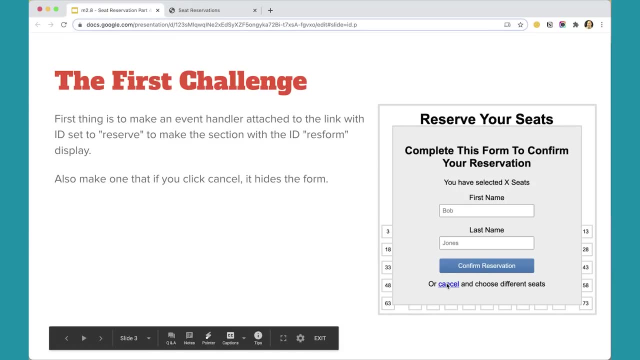 this button. I want this form to pop up and be displayed, And then on the form itself is a cancel button that if you click that, I want the form to be canceled and to be hidden again. So your first challenge is to make two event handlers for these two items: one for the button at the top of the 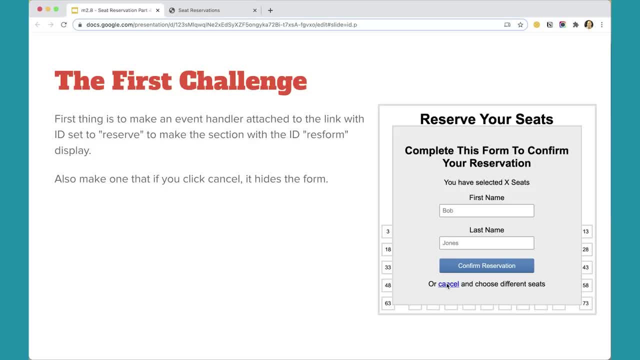 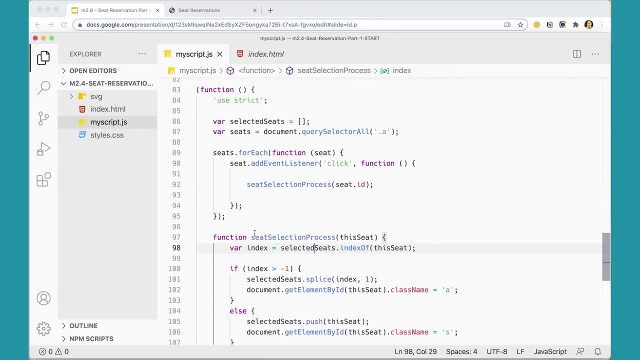 page and one for the cancel button. That will either set this form to displayed lock or display hidden. And these two event handlers could go really anywhere on the script. They could go over here, they could go anywhere. you could just put them at the bottom here. I'm going to put them here before the closing. immediately invoked. 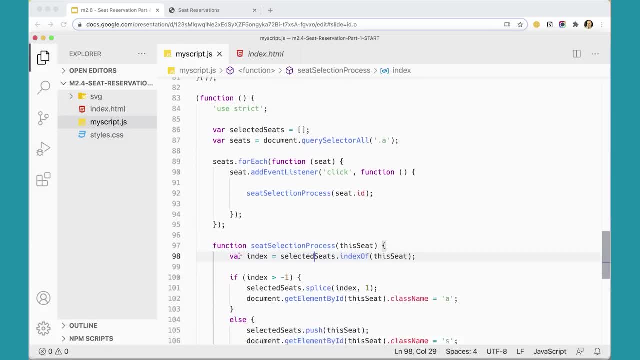 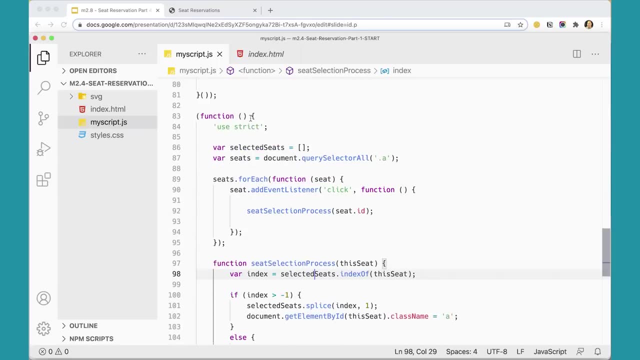 function just after the part that we did here, but they really could go anywhere. But I am going to keep them inside. I'm going to keep them out of this closure that I have here, because I think that that helps keep things clean and keeps everything out of the global scope. So I'm going to stick them in there, but you 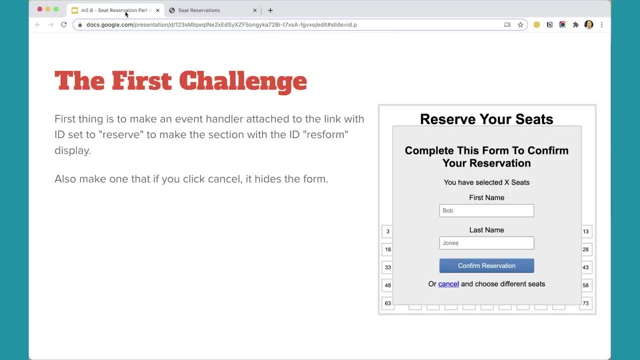 really could put them anywhere. Okay, so see if you can write that part for yourself. There's just two simple event handlers that are attached to IDs that will set this element, this entire thing, this entire section, to either display, block or display none. And then we'll look in the next video to see. 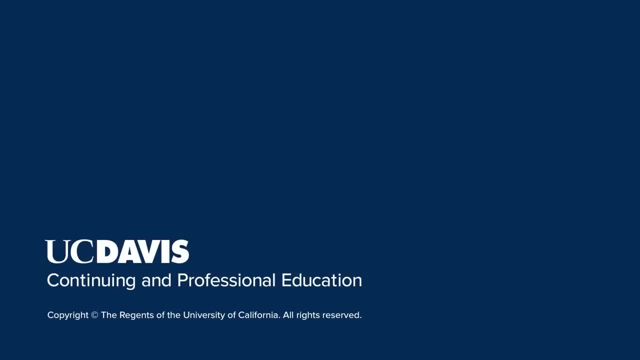 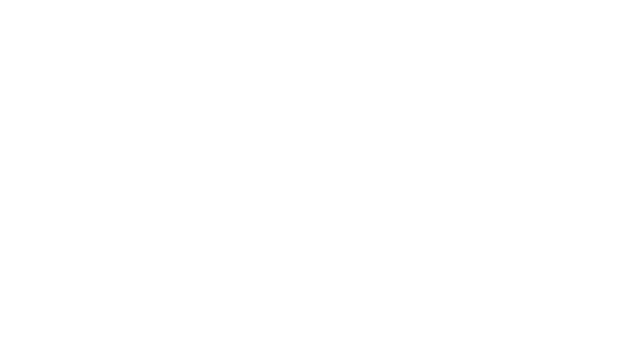 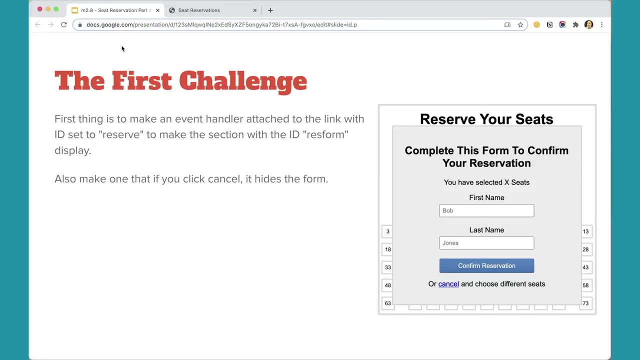 if you came up with the same thing I could up with. Were you able to do that challenge? The challenge was to write to event listeners, And let's see if you were able to do that. This is what I came up with. So I have an event listener. 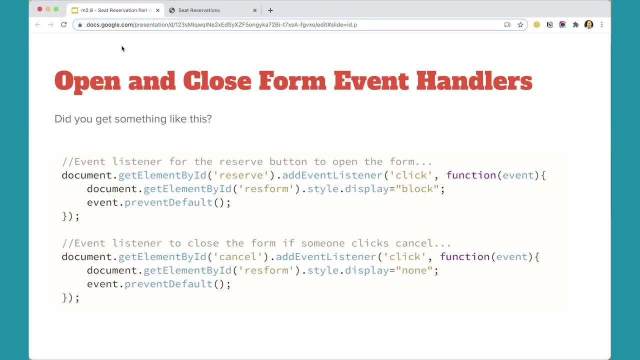 for when you click the reserve button which sets that ID for that form to display styledisplay block, And then for the cancel button which sets the style display to none. I'm also doing event prevent default in here, probably not 100% necessary, but it's a little bit helpful. 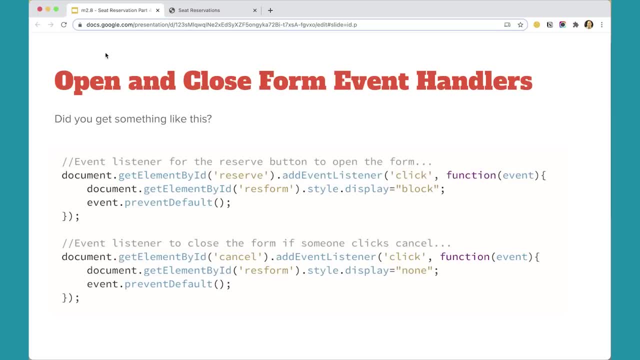 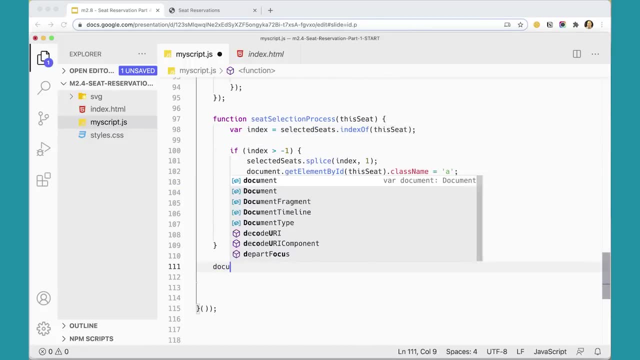 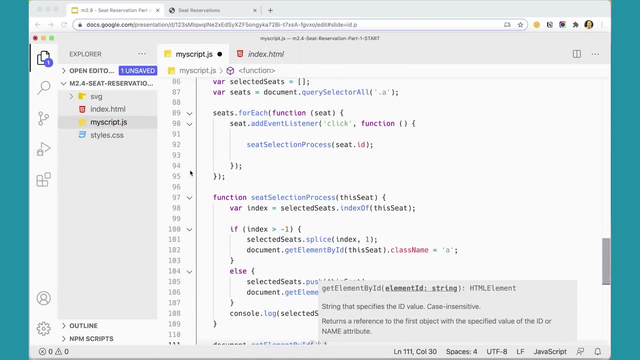 And I'll show you why in a minute here. But let's go ahead and get these into our code over here. So down here I'm just going to add documentgetElementById And the ID I want to get is the ID for this button over here. 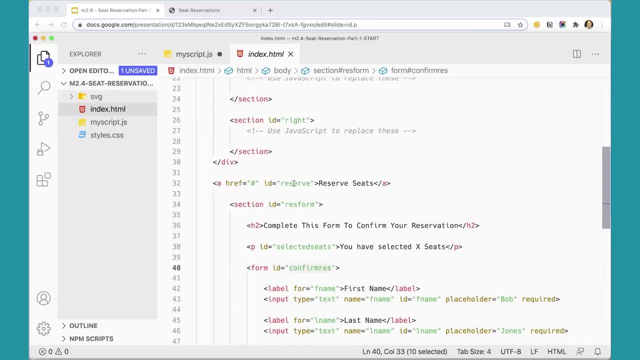 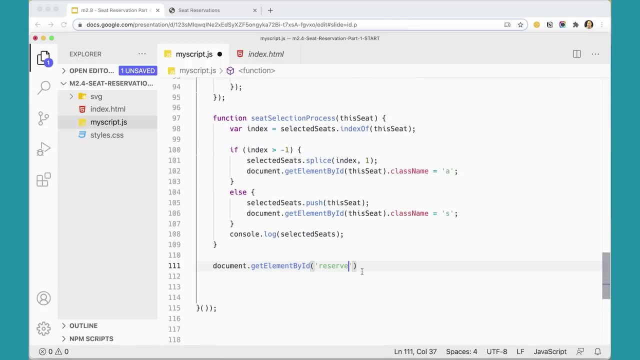 This reserve button here. So that's the ID I want. So I'm going to get that ID- getElementById reserve- And I'm going to add event listener to that button And when you click it, we're going to run a function like so: And what is that function going to do? 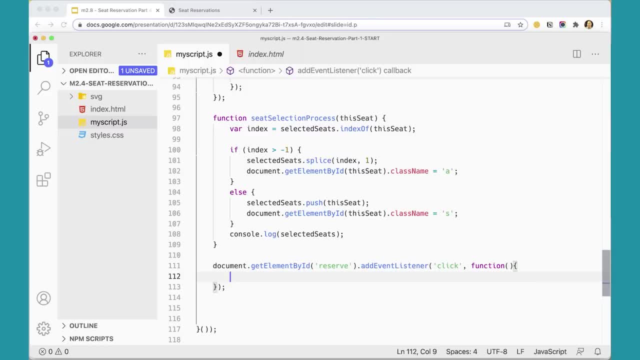 It's going to say: okay, first of all, we're going to pass in the event object here, Event object, and we'll say eventpreventDefault. I have that at the bottom in the picture that I showed you a minute ago, but it doesn't really. 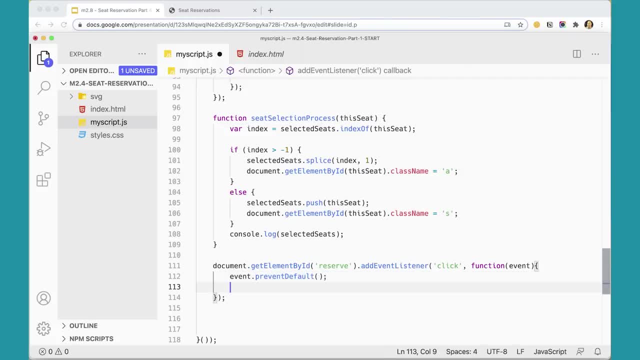 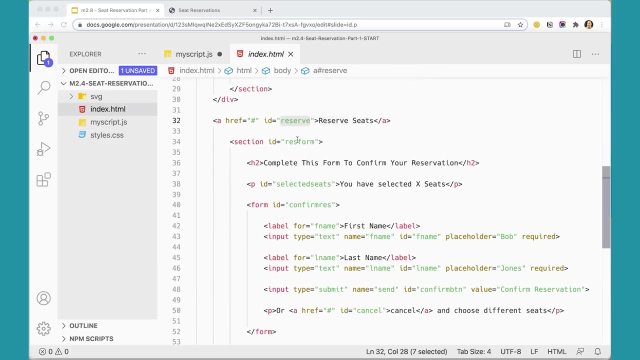 matter if it goes at the top or the bottom, And then, and then we're going to do okay, documentgetElementById. And the ID I want to get here is this: form, Res form, This entire section, which includes each, not just the form, but the entire section. 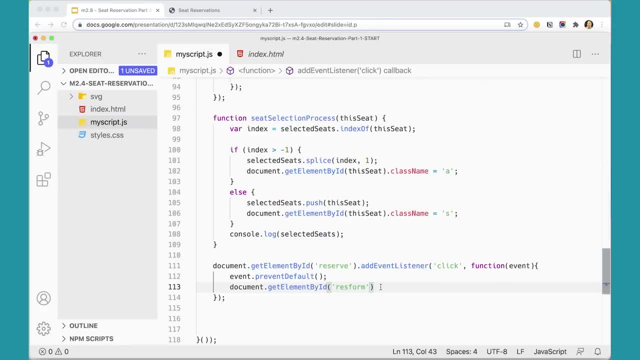 So we're going to get that entire section res form and set it's styledisplay to set that equal to block. I'm going to put that in single quotes just to be consistent. I think it's about block. There we go. Alright, so we're going to do that, And then we could do. 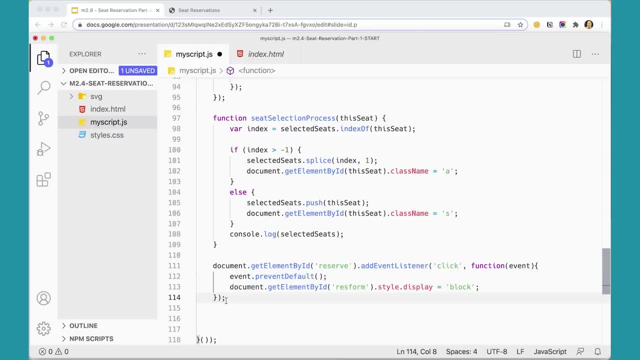 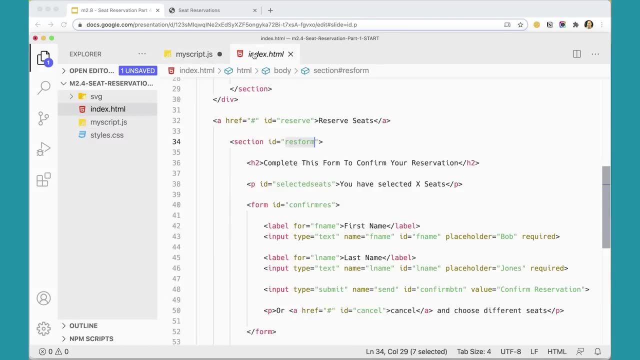 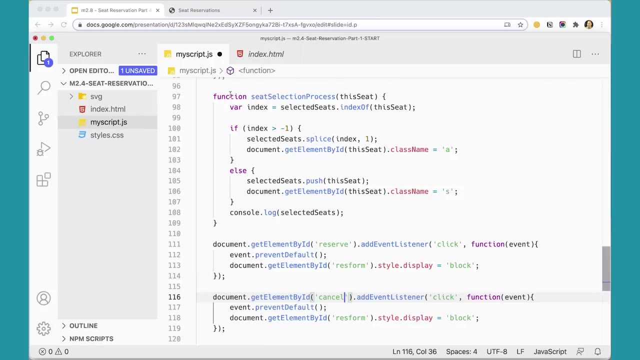 the same thing And you know, rather than typing it all over again, I'm just going to copy and paste this And, up here, change this to cancel, which is this button over here, IDCancel that anchor tag there, And I'm going to then set it to display none. 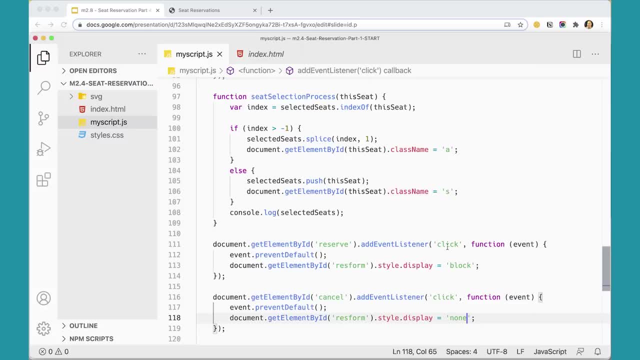 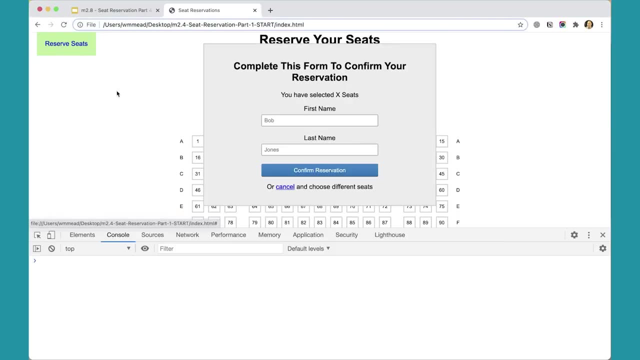 So that will hide it again. All right, let's test these two things. So if I come over here and refresh the page Now, if I click on reserve seats, that thing comes up. If I click cancel, it goes away. 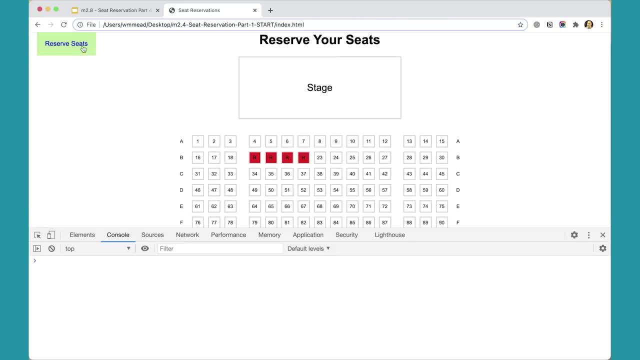 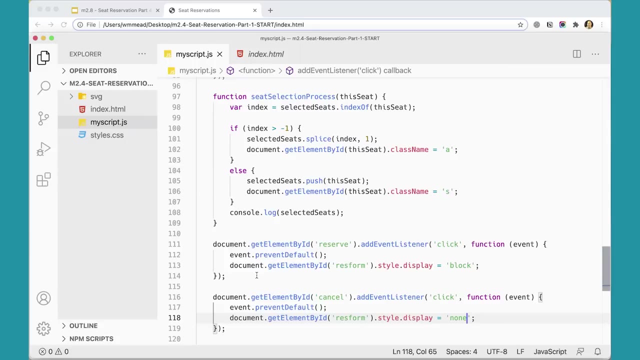 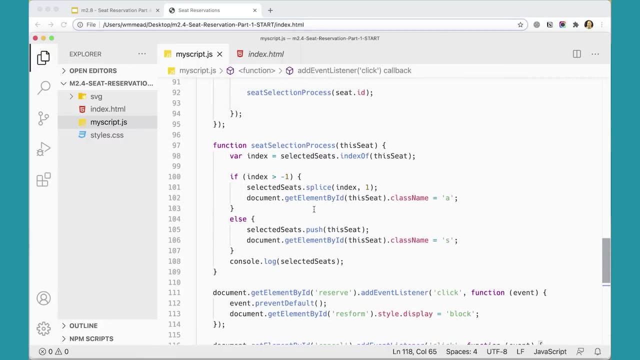 So that that piece of user interface is working is working. now you might wonder why i need the event prevent default here, these buttons. if you look in the html, they're really just anchor tags and they could be buttons. but buttons can be difficult to style. anchor tags are a little bit easier to style, so they're anchor tags over here. 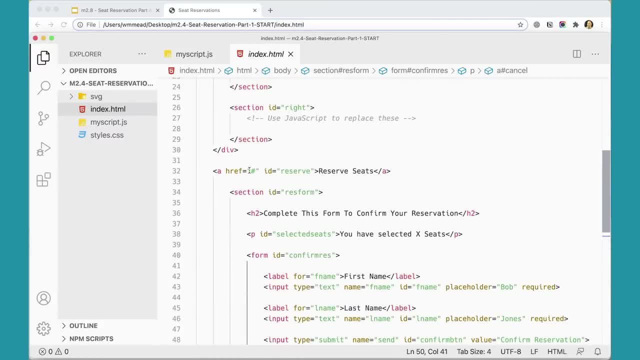 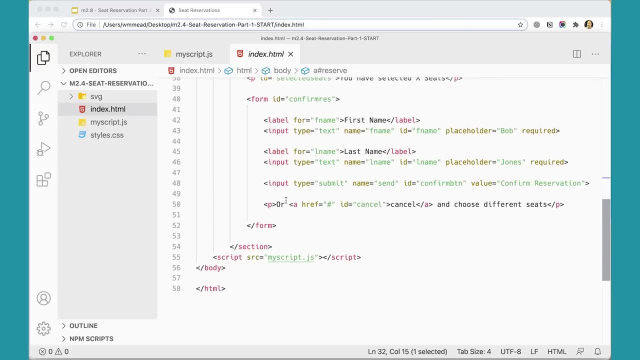 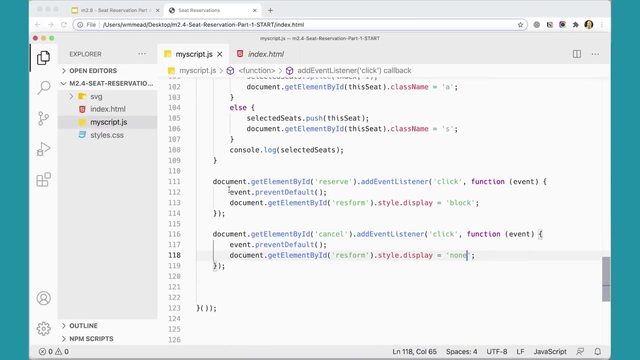 this is an anchor tag and it has as a url this href. if you're going to have an anchor tag, you have to have an href, and the href is equal to pound, and same thing down here with cancel. we've got a pound there, so if we were to turn off the event, prevent default stuff in here. 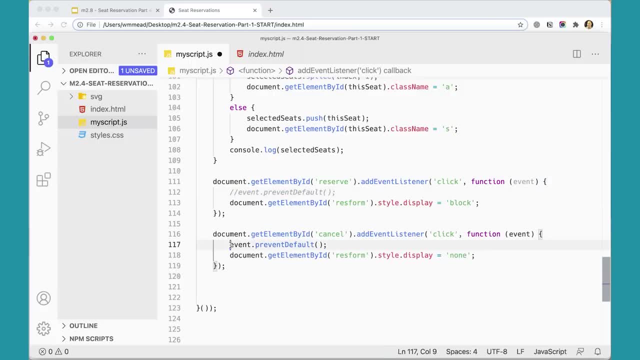 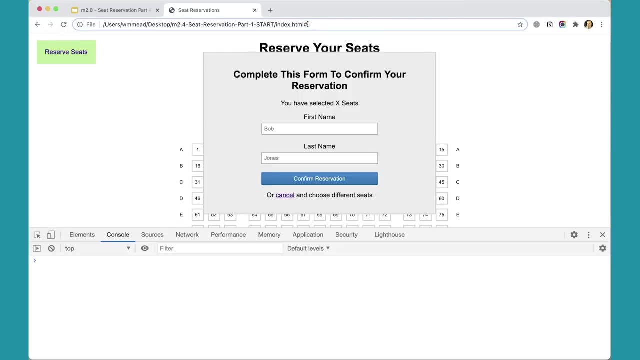 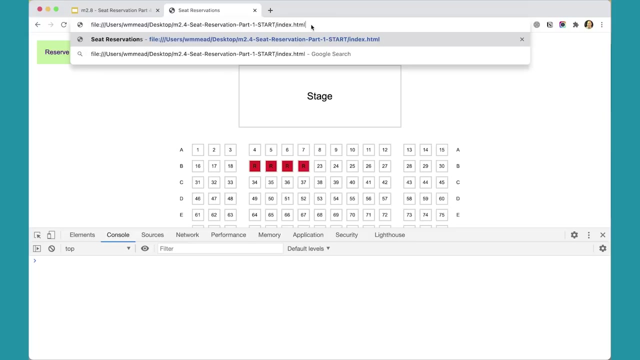 those hashtags end up up in the url when you click on these. so now i get the hashtag up there and you'll notice the page is actually doing a little bit of a reload when you do that too. but um, so just to get rid of that pesky hashtag there. i don't really want it there. 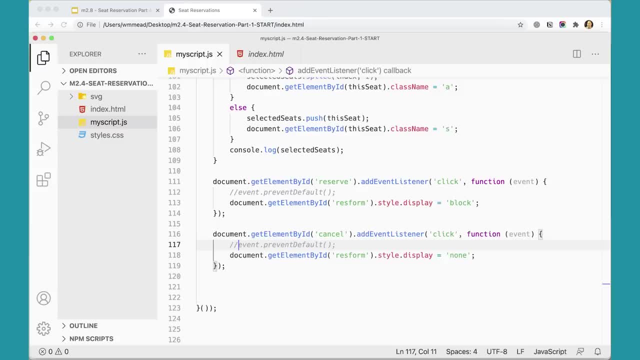 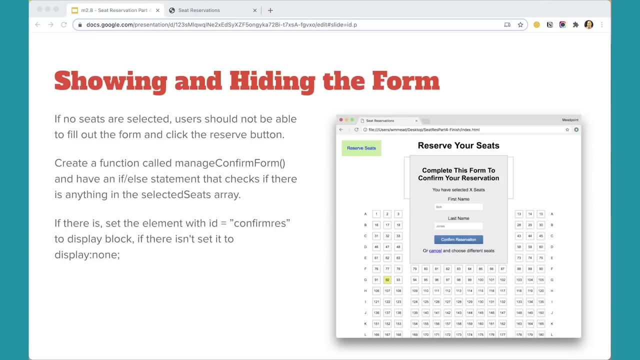 um, i think it's better to have the event prevent default in there, because it is actually trying to follow that link and whereas if we put event prevent default and pass in the event object here, then it doesn't try to follow that link. now that you have that working, what we need next? 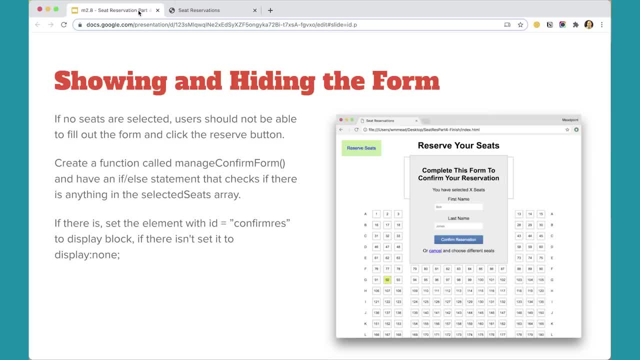 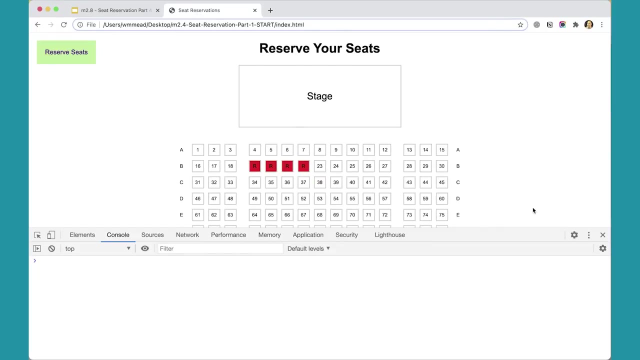 is a function called manage control, and what this function is going to do is it's going to handle whether or not our users can actually confirm, can actually make a reservation or not, based on whether or not they have anything right. so over here, notice, it's a little bit weird if i were to just come to this. 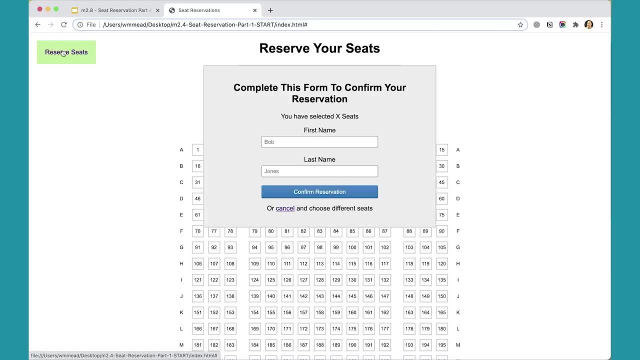 page. what if i just clicked reserve seats? what if i just click this button and i get this form to reserve some seats? i shouldn't be able to put my name in here and click the confirm reservation button if i haven't selected any seats. so but it's possible for users to come here and say okay. 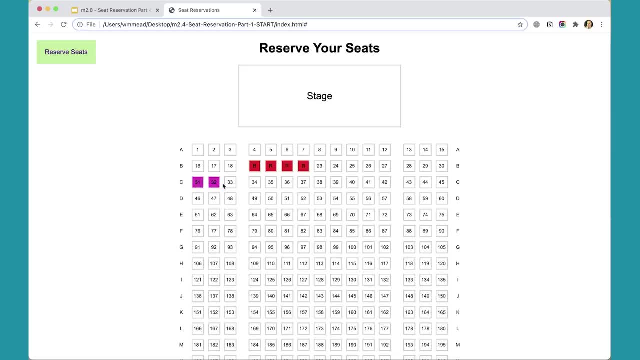 i want to reserve some seats without actually clicking on some seats to reserve. so we want to make it so that this form, this part of this page that actually has the form in here, does not display if the user does that. so if the array is empty, we want to run a function that says: 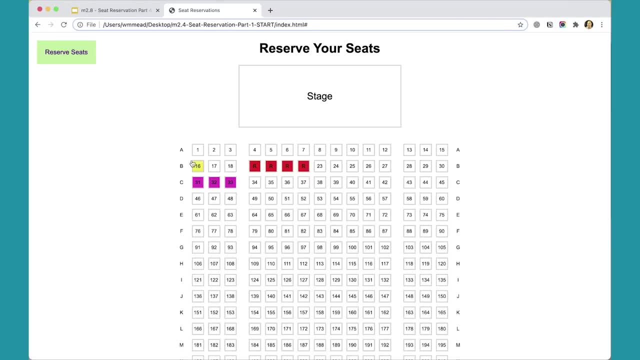 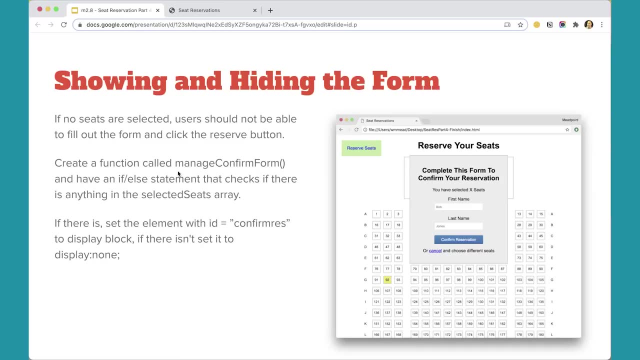 confirm that. that's a function called manage- confirm form that will hide that part of the form. so see if you can do that piece on your. so we're going to create a function called manage- confirm form. it's going to have an if-else statement in it that checks if there is anything in the select and seats array. 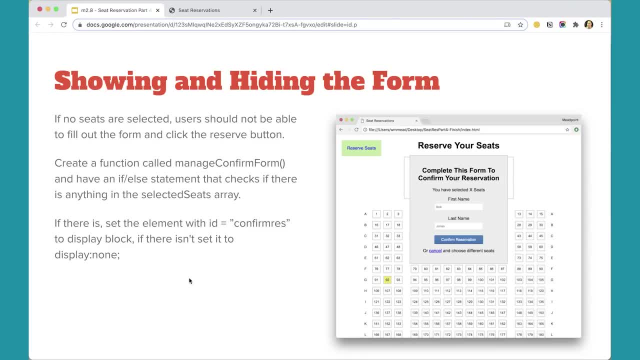 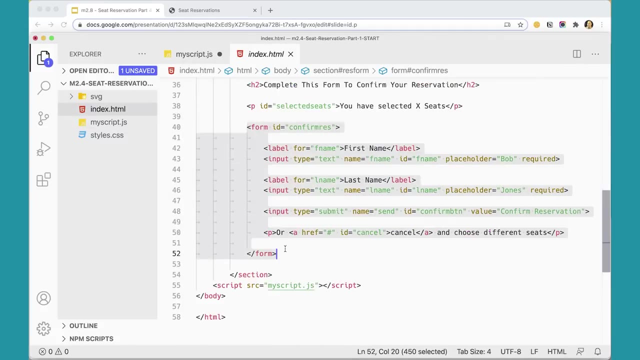 what is the length of that array if it's zero? if the length is zero, then set the element with confirm res, which is, if we go back to the html here, that's this form. we're going to set the form to display none, so that you'll still get the little. 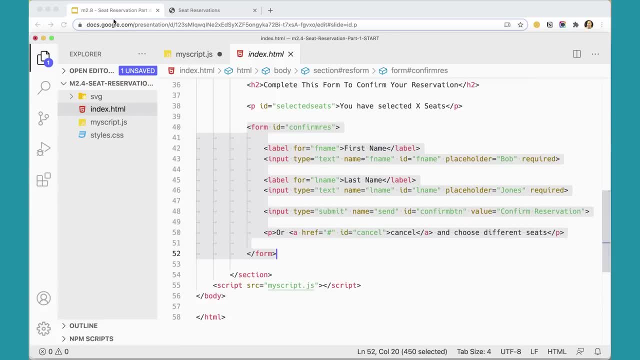 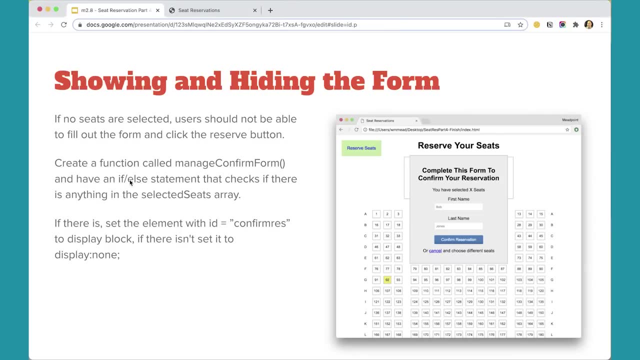 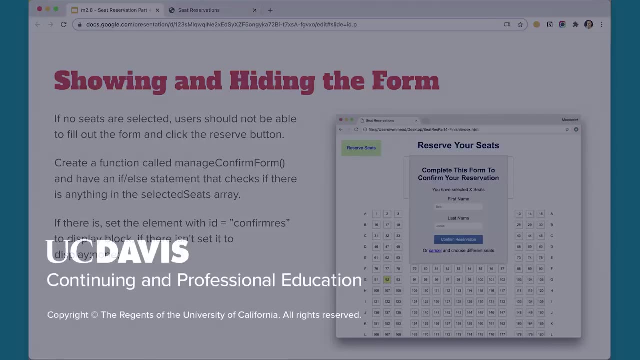 pop-up, but you won't see a form in there. if that makes sense, um, okay, so we'll set that back to display none and um, we'll set it to display block. if if there is something in there, okay, great. so see if you can do that on your own. 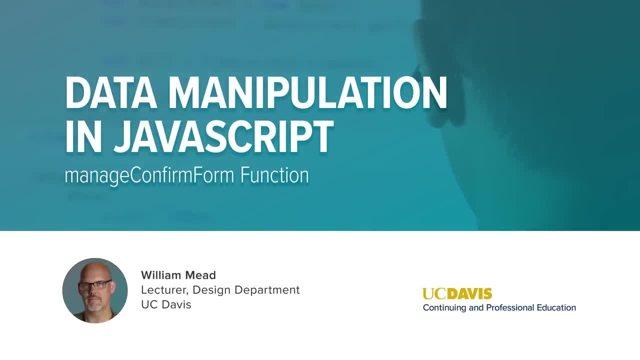 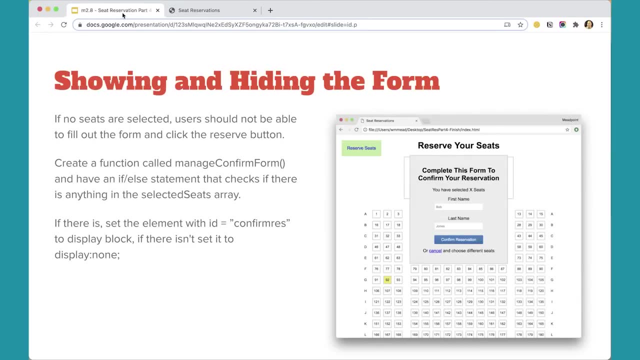 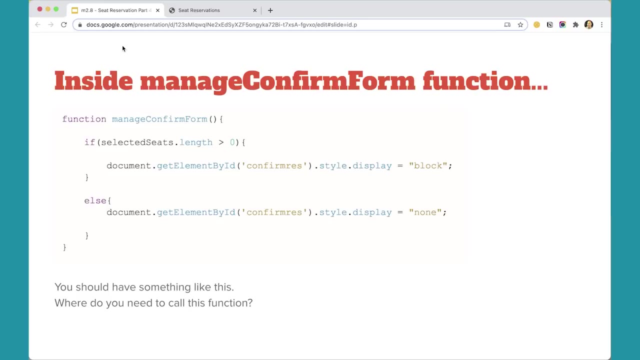 were you able to do this? we're able to solve this little micro um challenge. uh, let's see what i came up with here. so this is what i came up with: manage confirm form. if selected seats length is greater than zero, then i'm going to make sure that the confirm is is set to display block. otherwise i'm 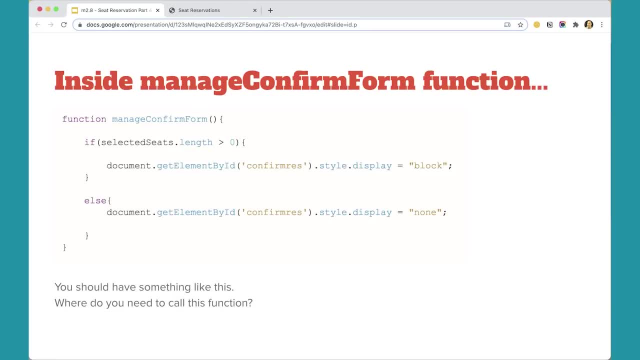 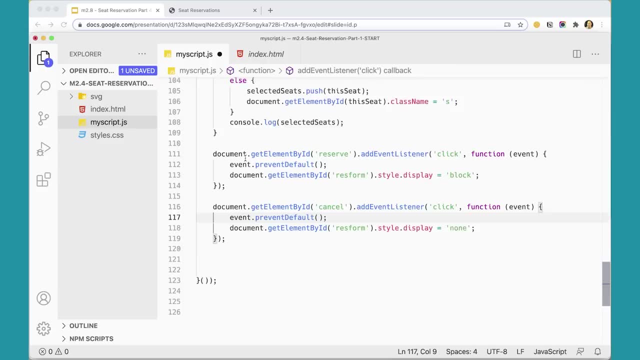 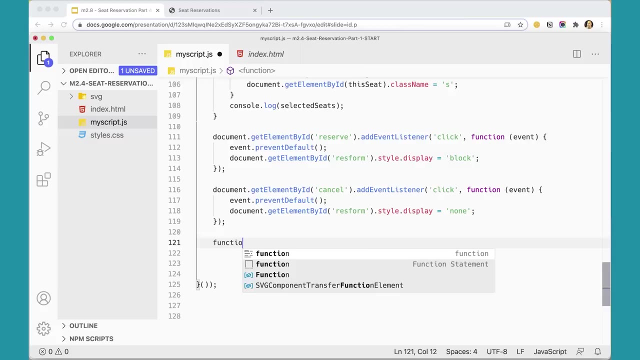 going to set it to display none. so let's go ahead and add this function over into our uh file, over here on our script file, and i'm just going to come down here and add function, manage, confirm form and i'm going to say if and what am i checking for? i'm checking for: 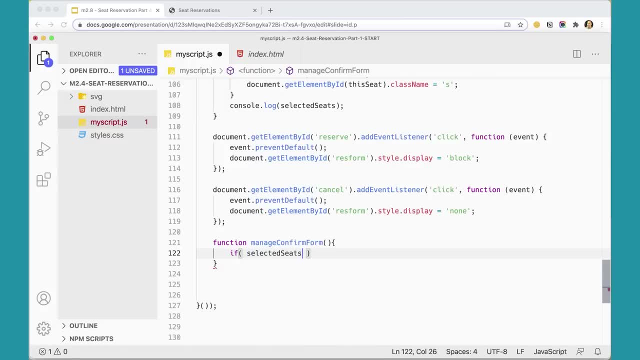 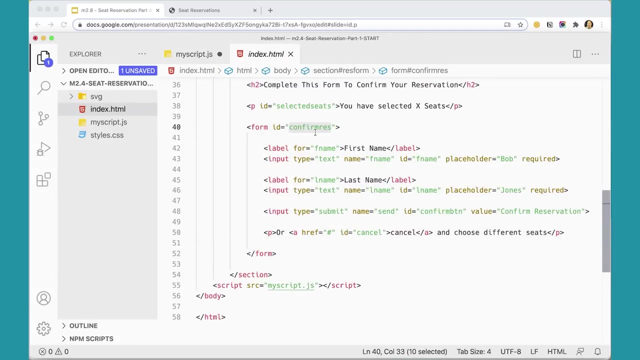 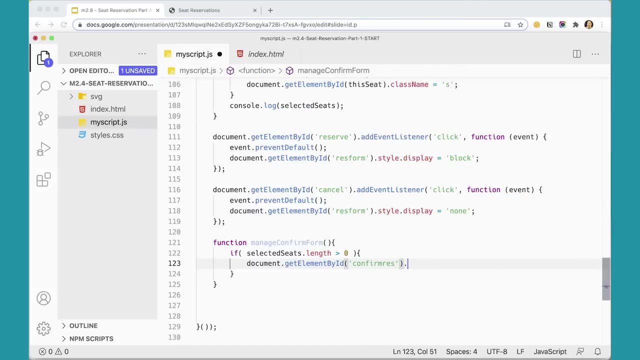 select selected seats: selected seats: dot length: if that's greater than zero, then i'm going to make sure that on my document dot get element by id. oops, confirm res. it's actually this id here, confirm res. just copy that, make sure i get it right. is set to dot style: dot display. 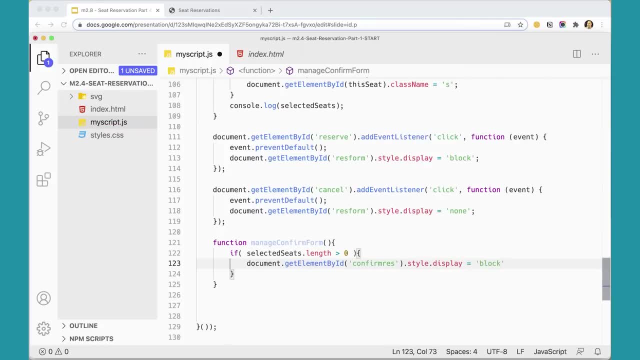 equals block. else, if it's not set to zero, then i'm going to make sure this thing gets set to display none. okay, great, so i have this function here. the next question is: where do i need to run this function? and i'm going to need to run it in a few different. 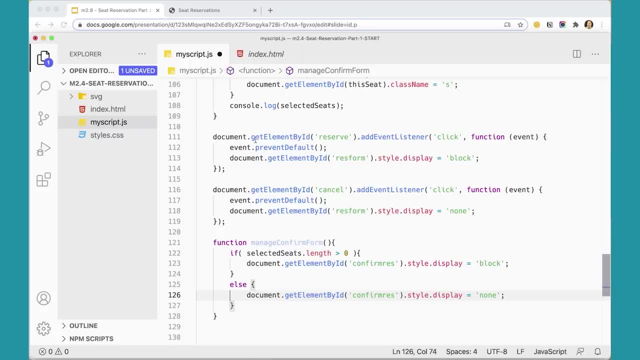 places and you'll see here. you know the the javascript is not that difficult. we're just setting elements to display or not to display. that's really all we're doing here. it's not a complicated javascript. but we have to really think about how the users might use this to support. 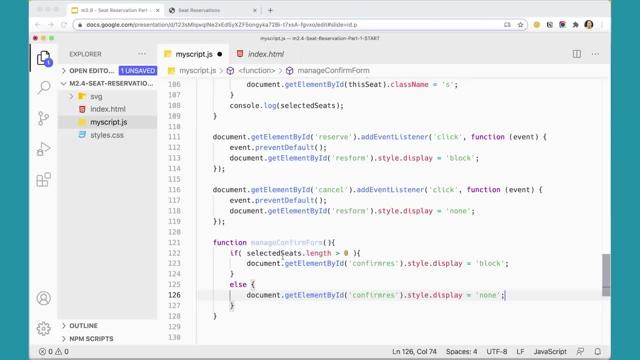 relationships, совет and sword on x-ray and we've had a lot of Luoan in application management and x-ray in dps tribute software and vanilla x-ray. alphard in the ms class to the ms class is a pre-mixed for that as a by default. it's a common step, which is to set a public leadership and find or suceder. 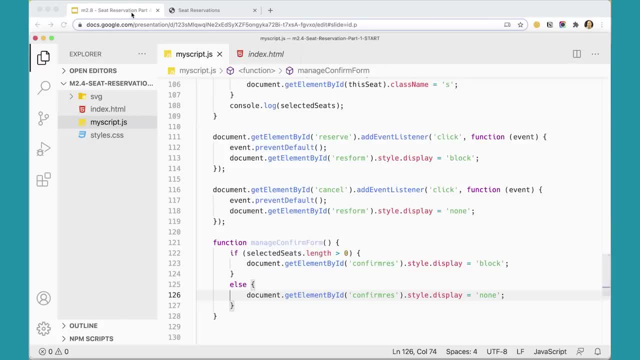 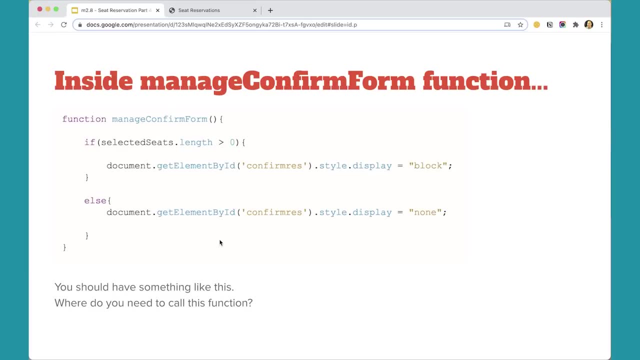 domain to some user when a script is designed, and that's where Pear and silk is feel like real health in the. the users might use this. So that's what we need to think about here. Where do we need to call this function? Well, we need to call it when the page loads, right, Because when the page loads, somebody. 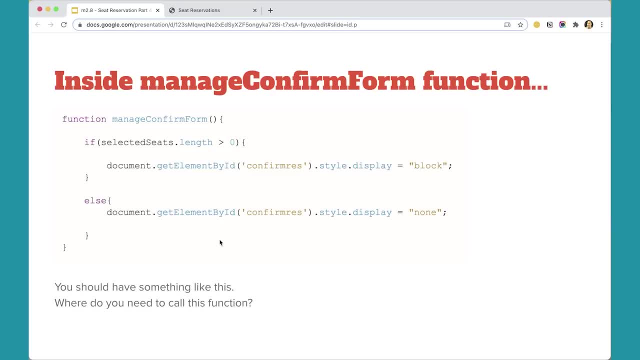 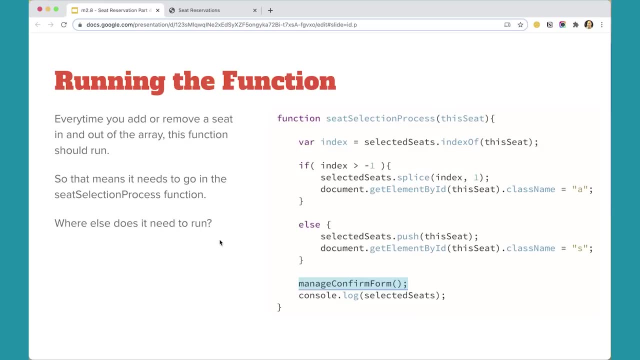 could immediately click that button, And there may be some other places where we need to run it as well. Every time you remove a seat in and out of the array, we need to make sure this function runs, because you could be removing the last seat, So we want to make sure it goes into the seat. 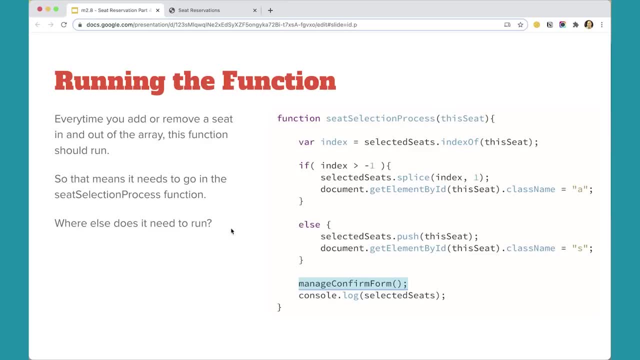 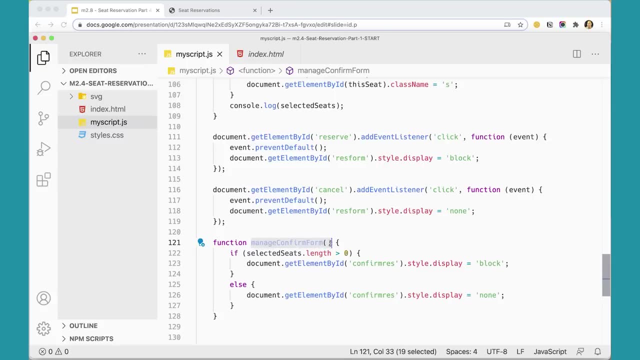 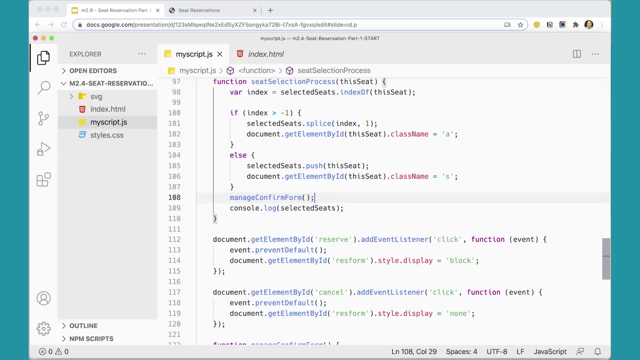 selection process as well. So let's go over and add it there. So I'm going to run manage, confirm form at the bottom of this seat selection process here And just run it there In case I've removed all you know. I selected some seats and then deselected them. I've taken, if I've 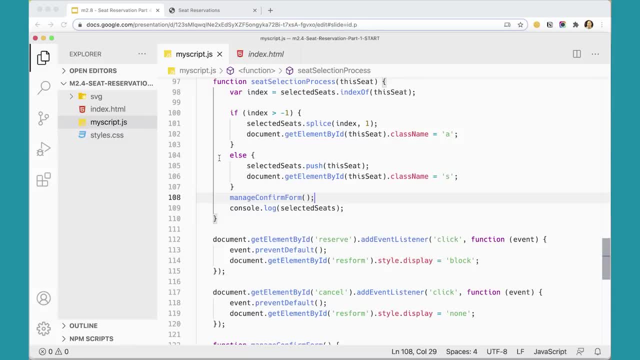 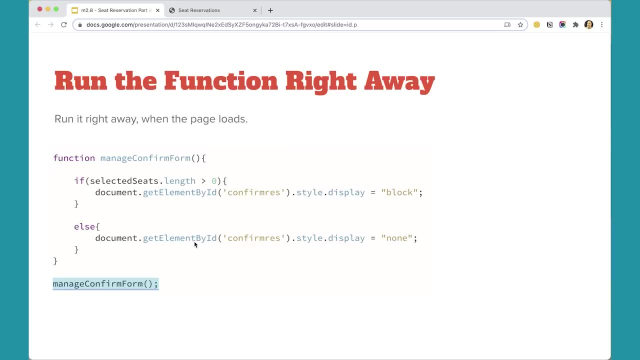 taken them all out. I can't, I shouldn't be able to reserve them. So that's one place I need to run it. And again, where else do I need to run it? I need to run it right away when the page loads. So 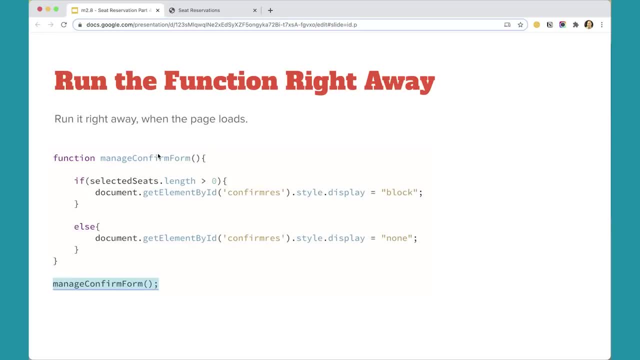 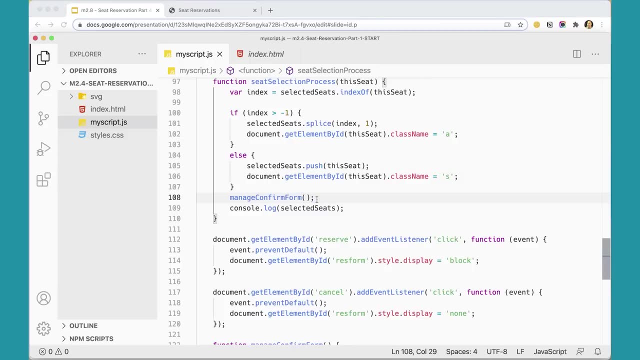 I'm going to just run it when the page loads right after I define this function, I'm going to run it there as well, Because it's possible that users could come in and just try to reserve seats right away. So I'm just going to run it here too. 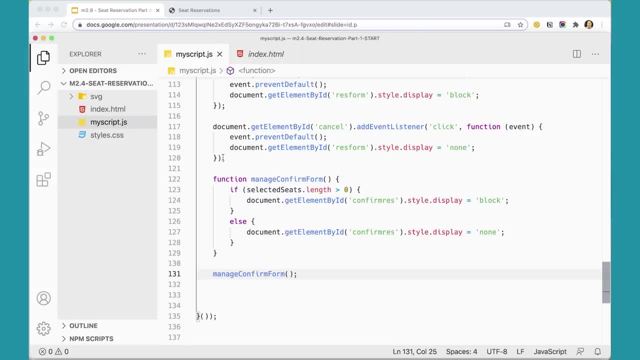 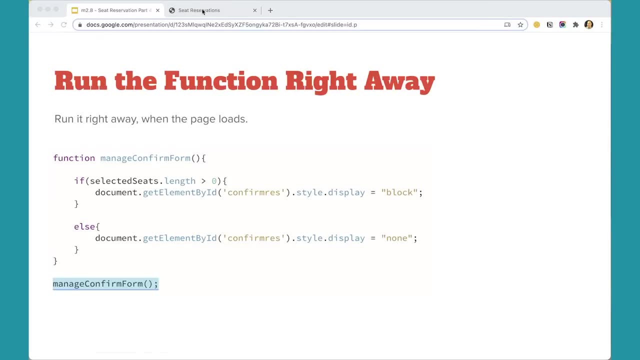 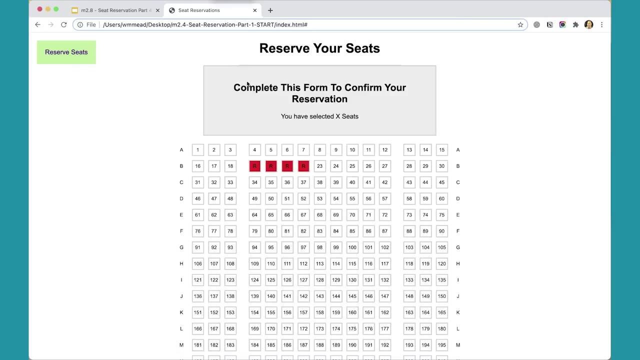 Okay, great, So we've got it in those two places. Let's test it. So if I come over here and click refresh the page, if I click reserve seats, I don't get a form. that's not going to work. So 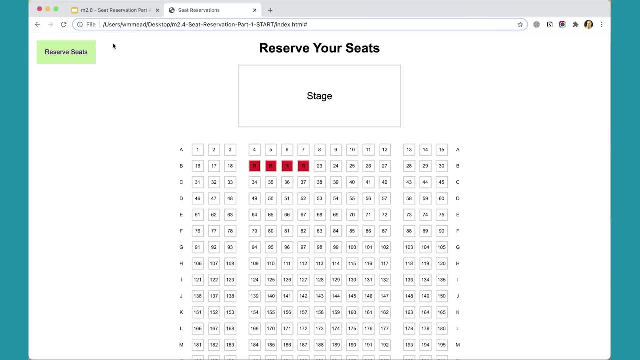 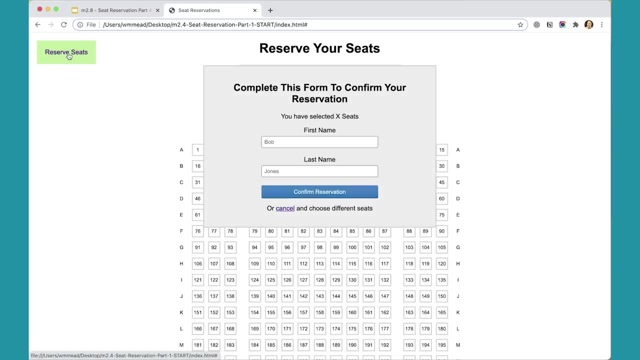 that's a problem. That's good. That's taking care of that problem. So now if I come down and select some seats and I click it, I get the form, And that's great. What if I select some seats and then 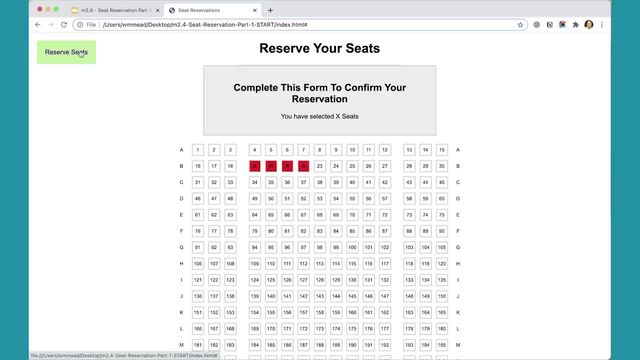 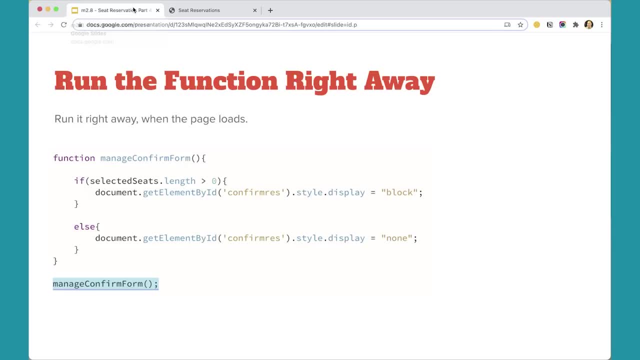 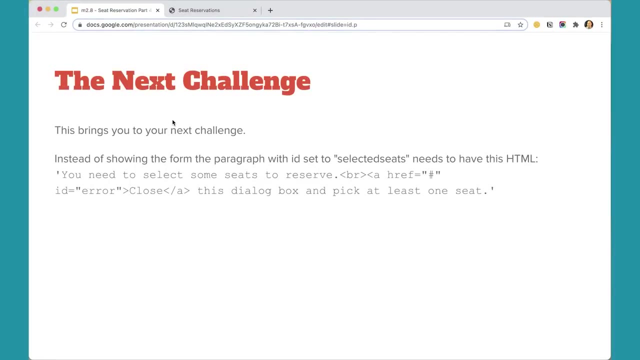 deselect them. Now. they're not in the array, the array is empty and I get that again. So that's great. So we've got that all in place there. The next challenge. this brings us to the next challenge. Instead of showing the, the form. 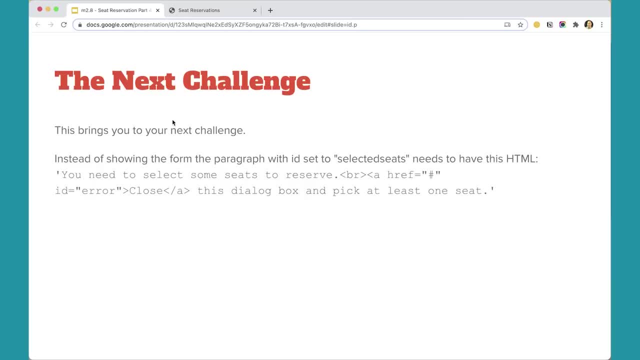 paragraph of the ID to selected seats. it needs to have this HTML. you need to select some seats to reserve and then have a break and have an anchor tag with an ID of error and then close this dialog box and click at least one seat. 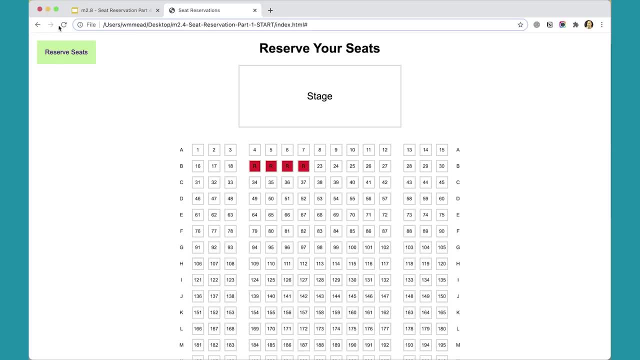 So we, because currently, if you come here and click this button, there's no good way of first of all, this doesn't make any sense. you've selected X seats. So we want to change that language to say you need to select some seats and then give them a close button to do that. 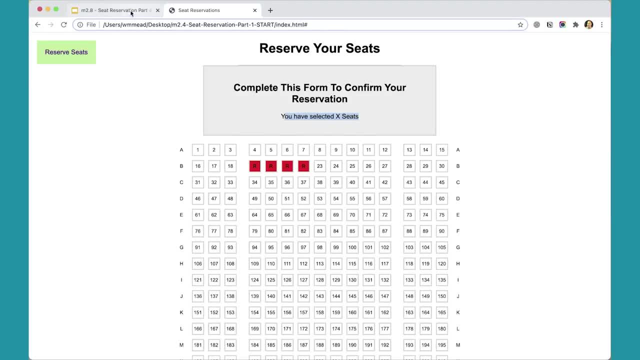 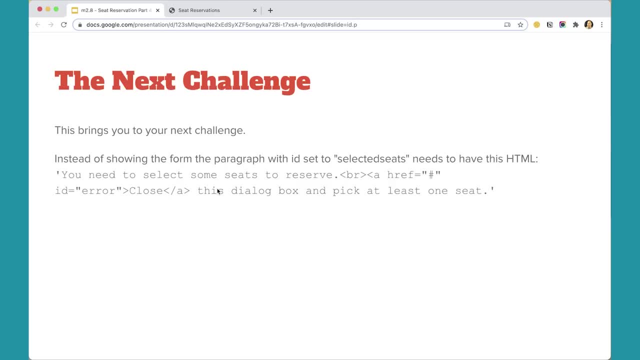 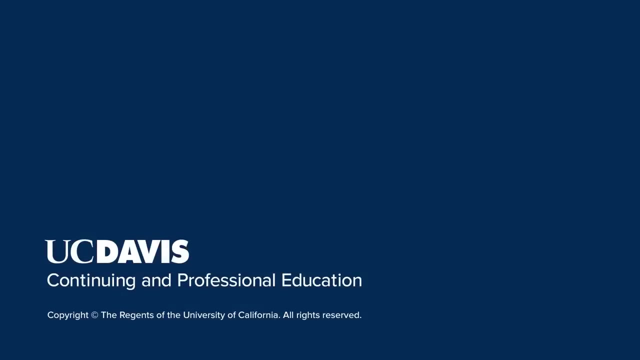 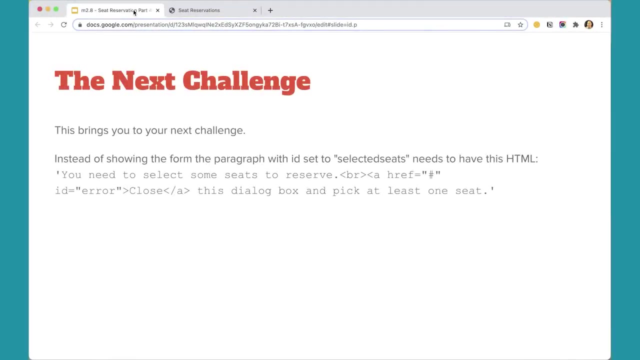 So see if you can figure out what we need to do to alter this part of the page so that it has that information in there instead, And then we'll look at my solution in the next video. Were you able to figure out this challenge, It shouldn't be too difficult. 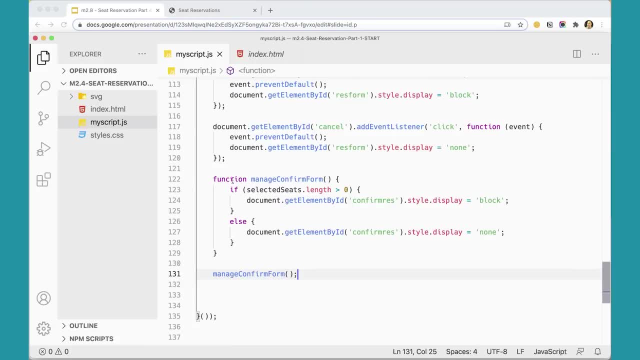 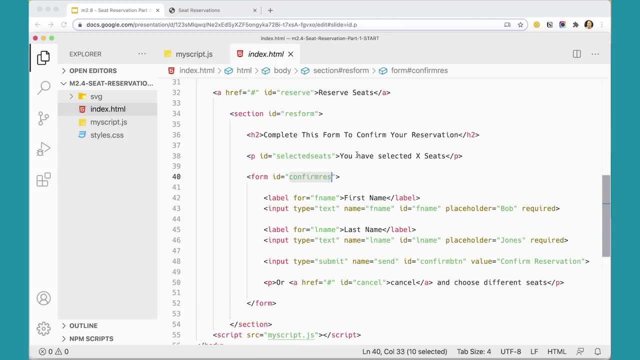 You can see over here in our HTML that if we look in here in the HTML, that what we really want to change is the value of this, the inner HTML of this paragraph. here And when do we want to change it? We want to change it if, if this thing is set to display none. 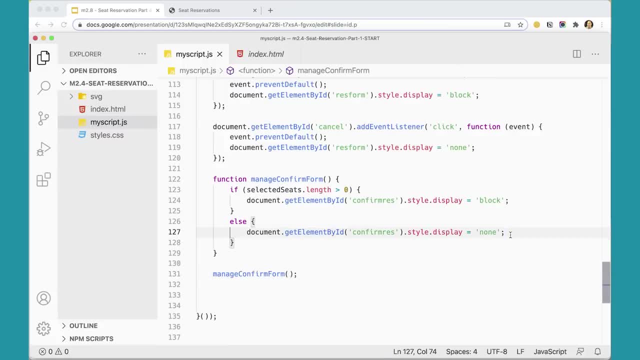 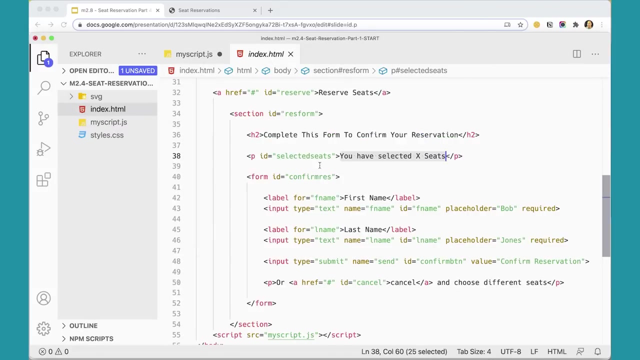 So that shouldn't be too difficult to do. All we need to do is do is document. if we do this, this is going to tell us if we will actually use this. you know, element by ID. Oops, I could type properly: document dot. get element by ID, And the ID that we want here is this ID over here, this. 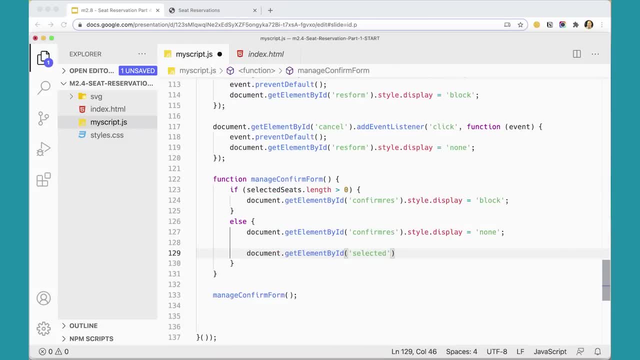 the id of this paragraph: selected seats. get that ID and change it. it's dot, innerHTML equals, and I'm going to just paste this in here, but you're going to have to type it something like that: innerHTML. you need to select some seats to reserve. I have a break and then I have an anchor tag with an ID. 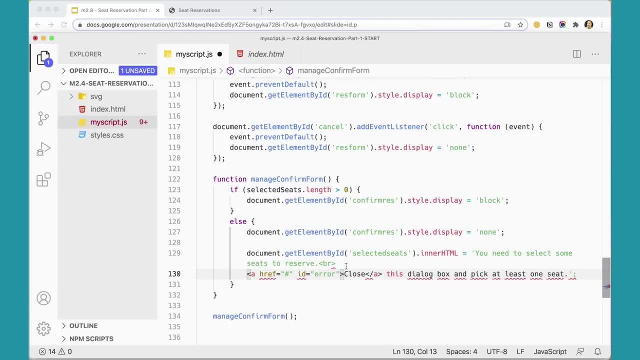 here that I'm going to unwind if you want. I guess I can't because weird things, but I have a break. I have an anchor tag with just a href there and an error close and then this: you know, close this dialog box and that's going to be a link to close. 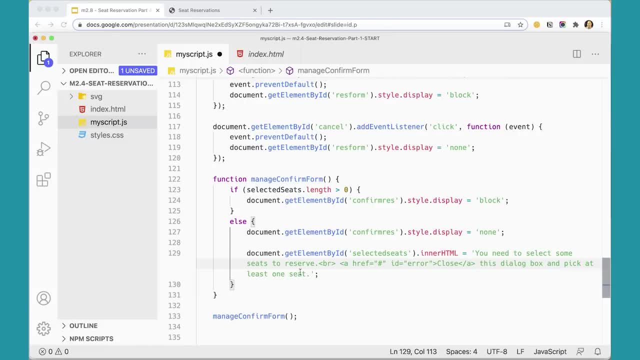 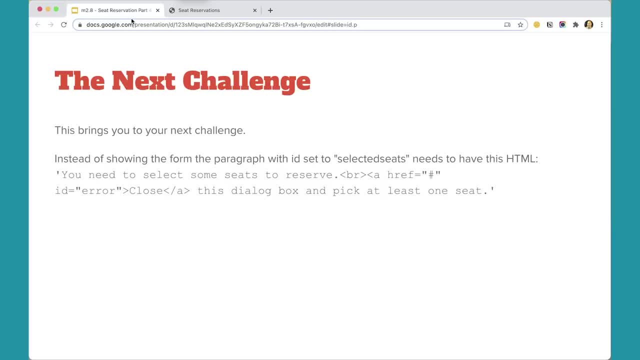 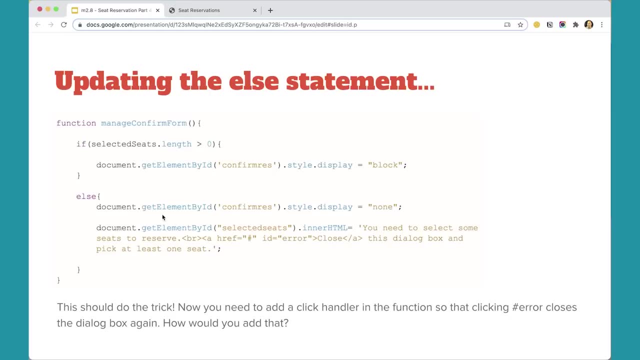 have over here. if we go back and look at our images here, this is what i came up with. document: get owned by these selected seats. enter html. you need to select some seats to reserve. great, that should do the trick. now you need to click it. add a click handler in the function. so. 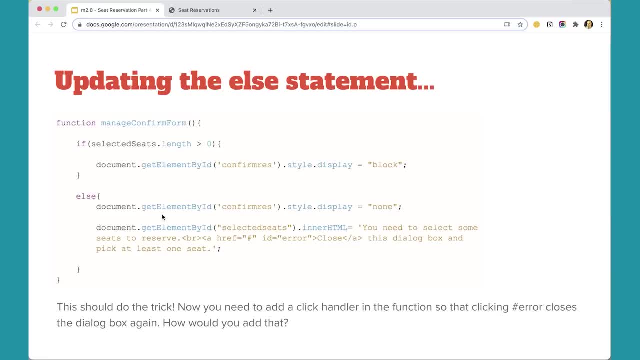 that clicking the error closes the dialog box again. so how would you do that? pause the video here and see if you can add that in, and then come back to the video and see what you can do, see if you did the same thing again. this is a pretty simple. 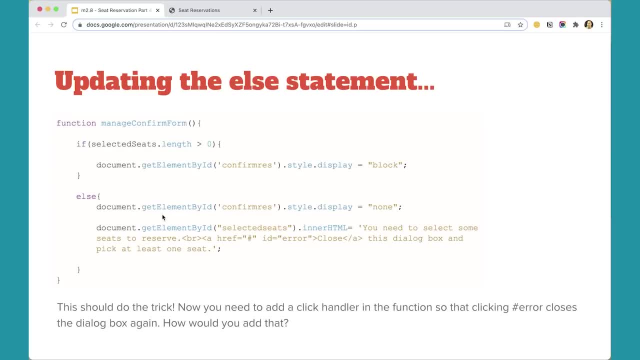 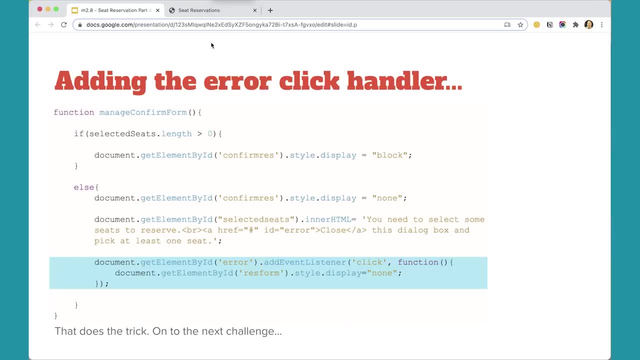 challenge here, so see if you can do it on your own. this is what i came up with. hopefully you came up with the same kind of thing here. document: get owned by the error event: listener click function. document: get element by id document: getorfacilegevercom. 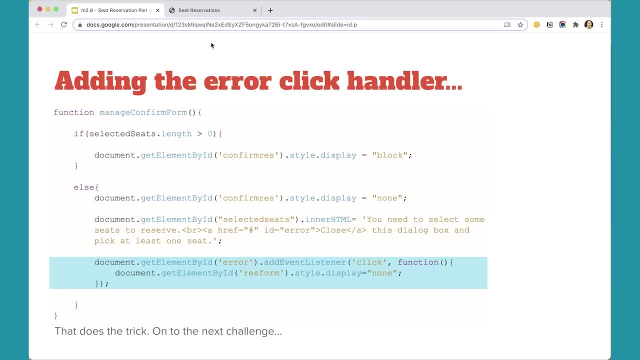 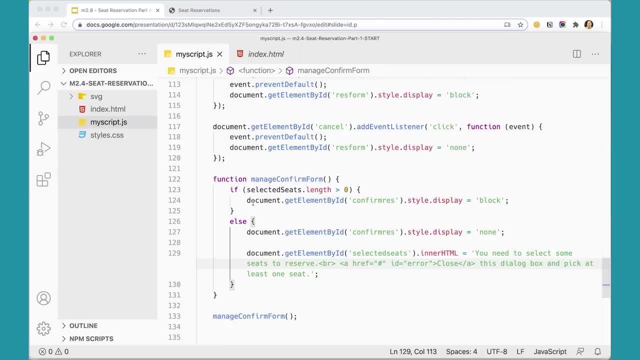 res form style display: none, so that's just hiding the entire res form again so that we can close it. and, uh, hopefully you got something like that, let's go ahead and add this over here. so down here i'm going to add document get element by id. the id that i want to get is this error: 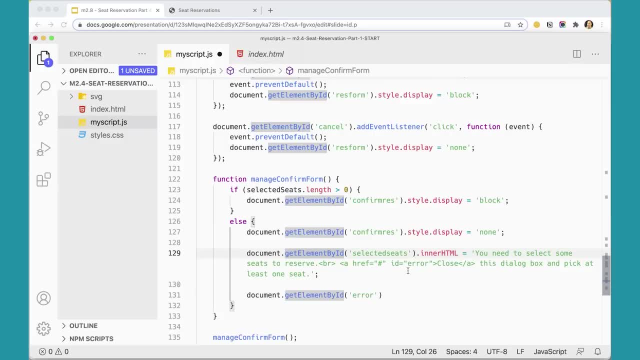 because that's what i'm clicking on. is the error that got set here? get that id dot, add event listener click, and then i'm going to run a function- parentheses, curly braces, semicolon there- and in that function i'm just going to say: document. it's really just. i don't even have to type it because it's really just this line right here. 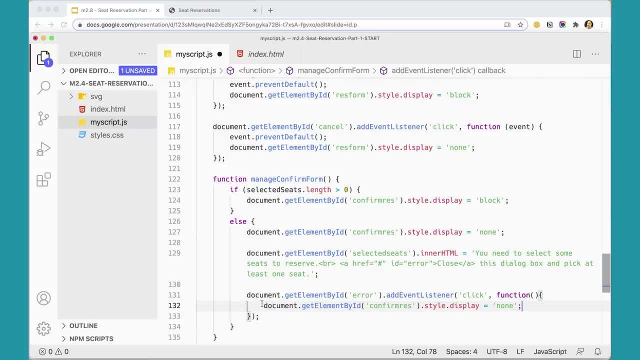 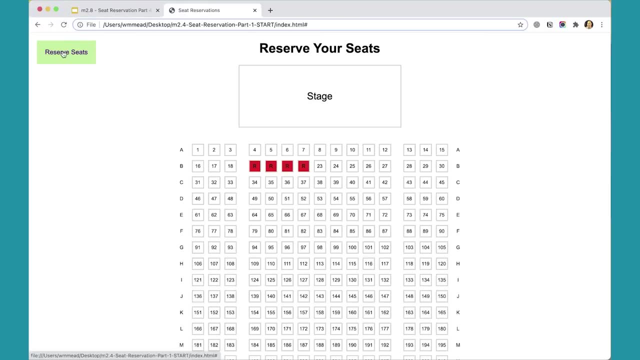 i can just paste that in. get element by id: display none, and that should take care of that. so let's go and test it. so if i come over here and click refresh, if i just click reserve seats, right away i get a dialog box. it allows me to close this. 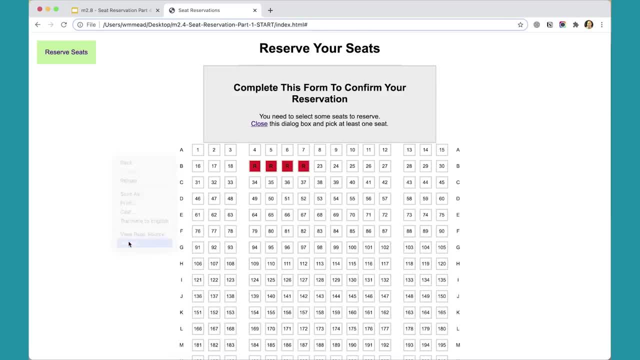 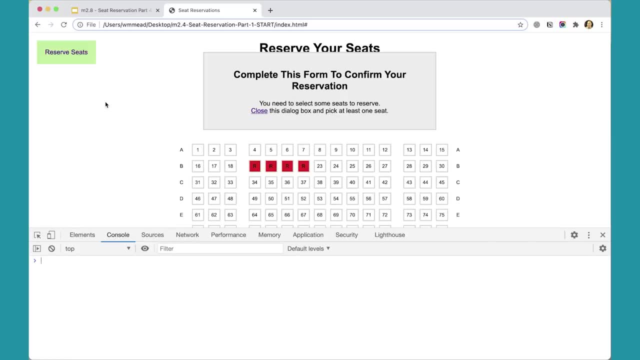 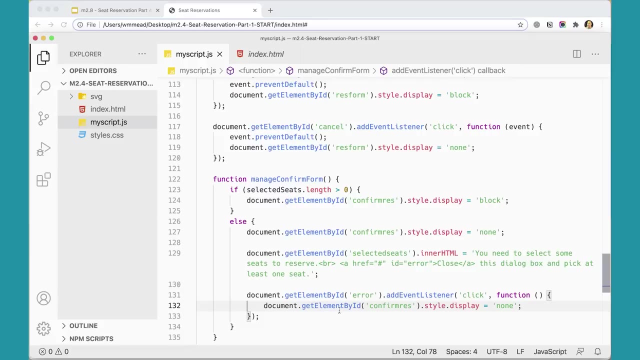 and it didn't work. i must have spelled something wrong. let's go ahead and inspect. i'm not seeing anything in my console, so i must have really spelled something wrong here. i'll go back to my previous menu. the next screen is: get element by id: confirm. oh, it's not this one that i want. 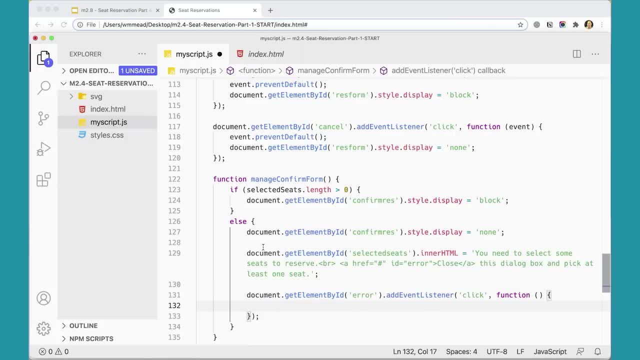 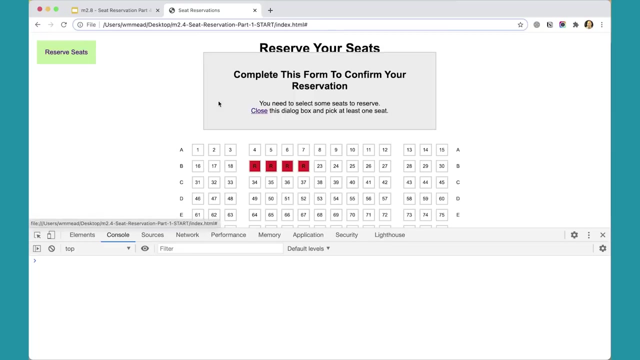 that was already set to display none, which is why it was doing nothing. i want this one res form display. no, let's try that. Observe seats, click close and that goes away. So that's actually working perfectly fine now. But you see, here you have to think carefully. 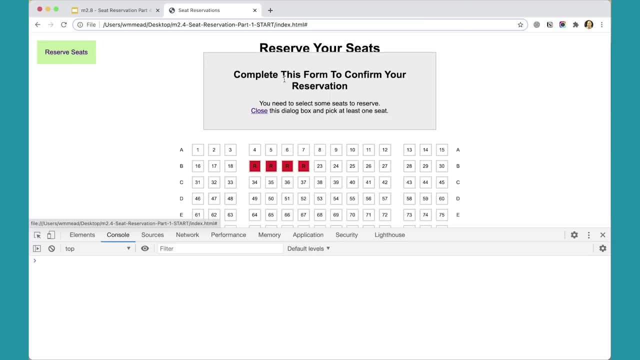 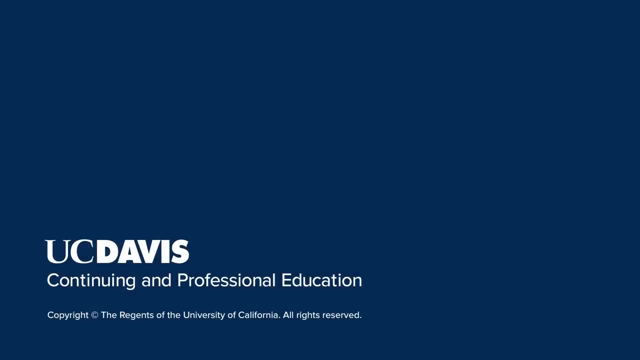 about the user interface and what users could do, and changing the contents of your interface so that it makes sense for what it is that users need to do in that context, And we'll be doing a lot more of that in this part. The next thing that we need to do: 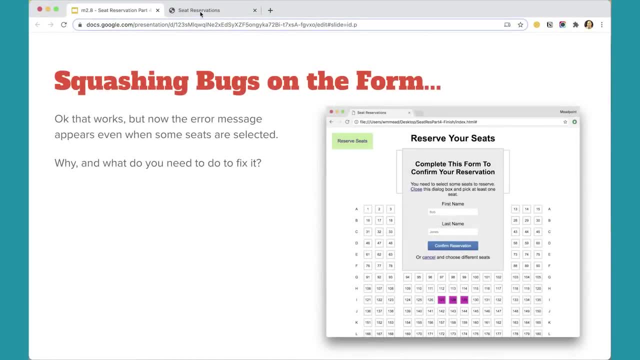 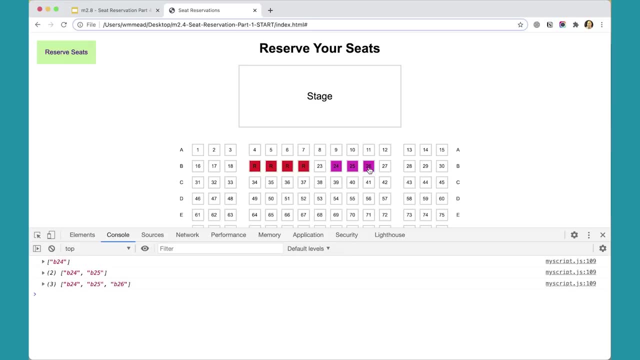 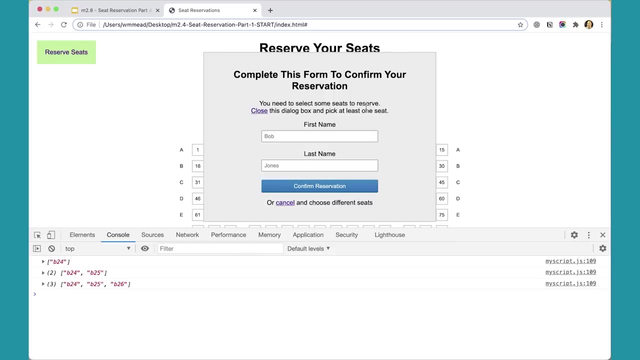 is fix some bugs that we have here And let's see if we can identify one over here. So I refresh my page. What if I select some seats and then click on reserve seats? I'm still getting this message here: You need to select some seats to reserve. 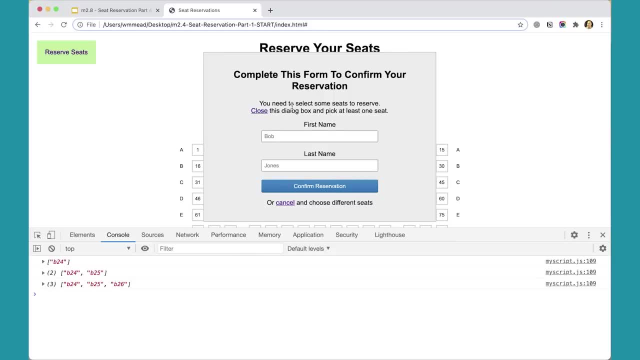 Close this dialog box and pick at least one seat. Why am I getting this? I did select some seats. That doesn't make any sense. What's going on here? Why is this message showing up? Can you identify what the problem is that's causing that? 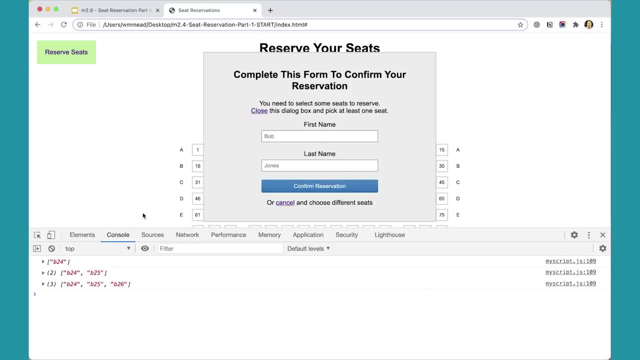 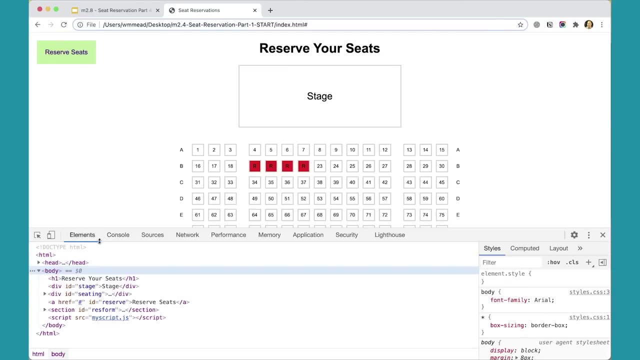 If we come down here and inspect- suppose I close this and just refresh the page- And then if I go to my elements over here and look into my reserve form down here, I just see I've got P selected seats. Notice, it says this right here. 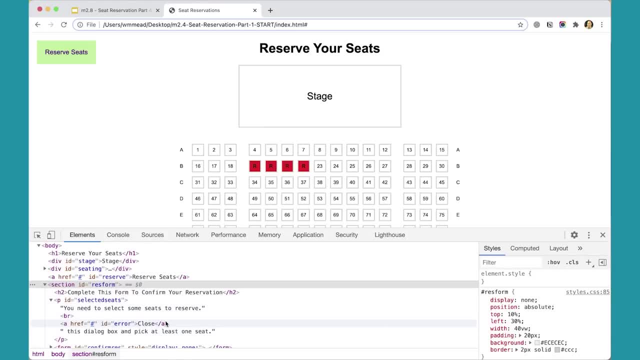 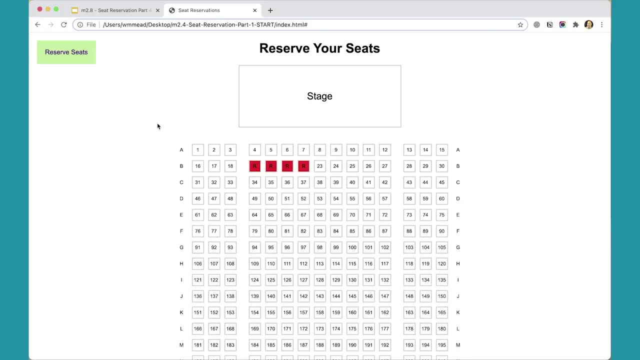 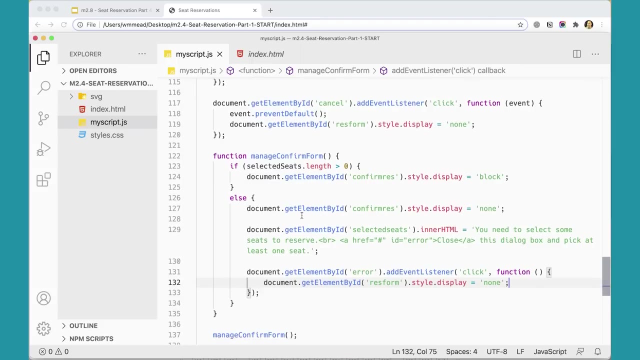 You need to select some seats. Hopefully you noticed that the reason why that's coming up, with it coming up right away, is that we're running that function, The function Managed- confirm form, when the page loads. So when managed- confirm form, confirm form. 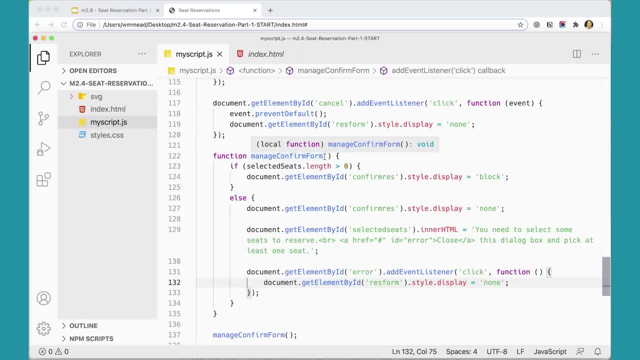 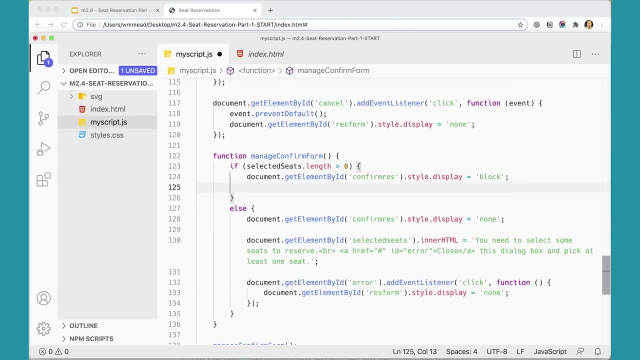 runs when the page loads. no seats have been selected, so immediately the confirm res is getting set to display none and that content is getting swapped out in the DOM. even though you don't see the form initially, it's getting swapped out when the page loads. so one way of dealing with this, and we can make it better, but for right now, one way of dealing. 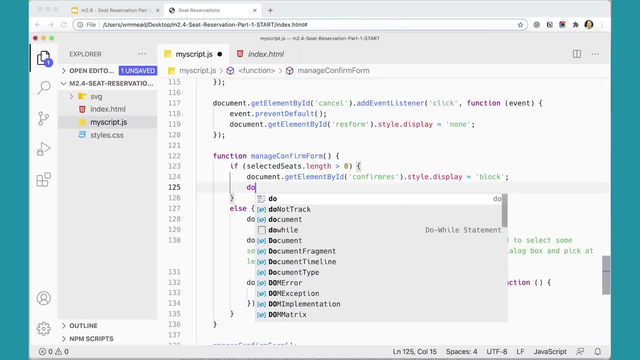 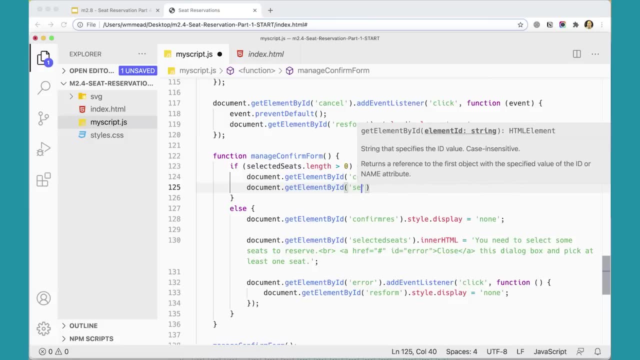 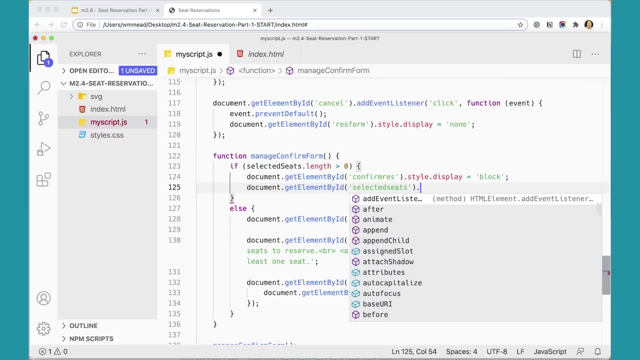 with this is to do appear document dot, get element by ID, selected seats. you're going to get that ID and set its inner HTML to. I'm just going to set it to. you have selected some seats and we're going to do that essentially if the nationals you set pk methods, the kind that makes 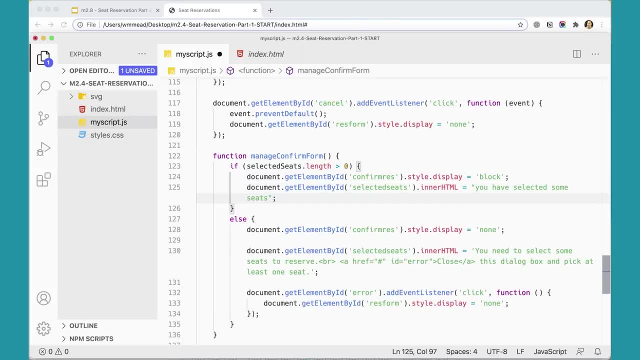 it so easy for you. if you guys have questions about it, try to figure it out as to how toito track to make this better, a little bit more useful. but at least now when, if the length is greater than zero, we can change that text to something that makes a little bit more sense. so let's go over. 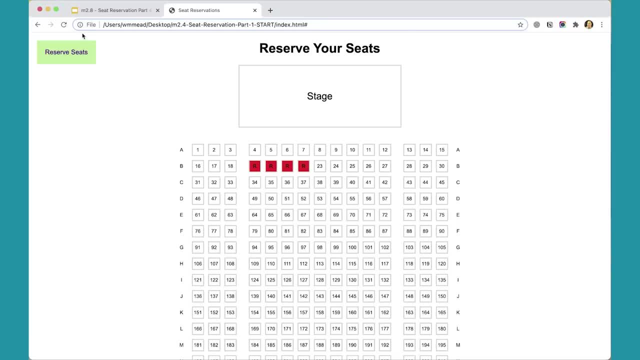 and take a look at what that does. so if i refresh this and then click on some seats and click reserve seats, it says you have selected some seats, be kind of nice if it said what seats you've selected. so we'll fix that, but at least we're able to get it so it doesn't have the error. 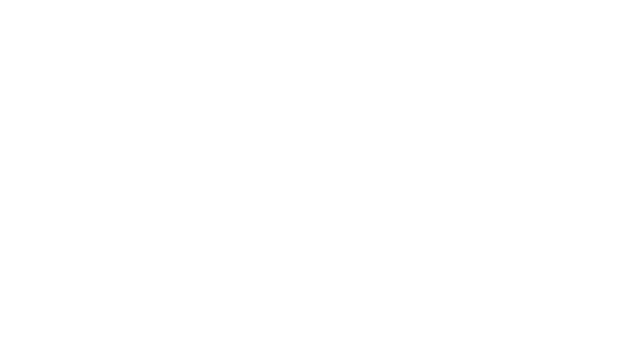 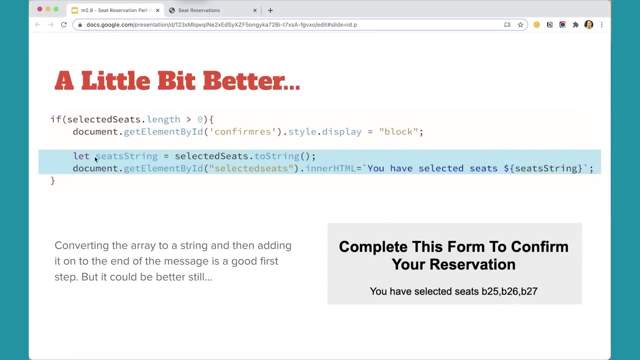 message up there. let's make that message a little bit better. here i'm going to use a variable called seat string and i'm going to have selected seats to string. go into that variable and then down here we can use: you have selected seats and then the seat string, so that that'll give us 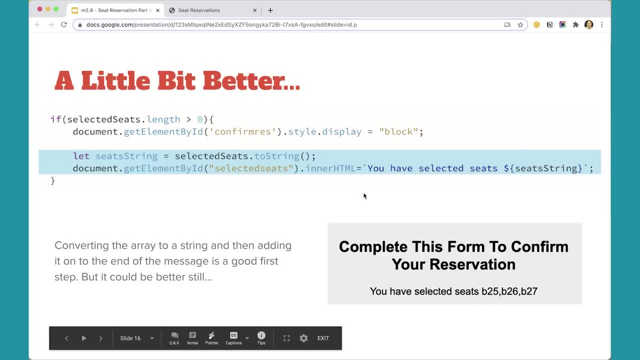 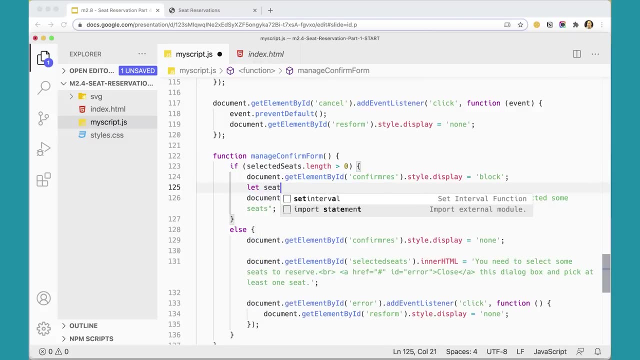 a string of seats kind of like this still doesn't look very good, but we'll fix that up in a minute to make it look even better than that. but let's do this first, just to get started on this. so over here i'm going to come in here, i'm going to say, okay, let seat string equal selected seats. 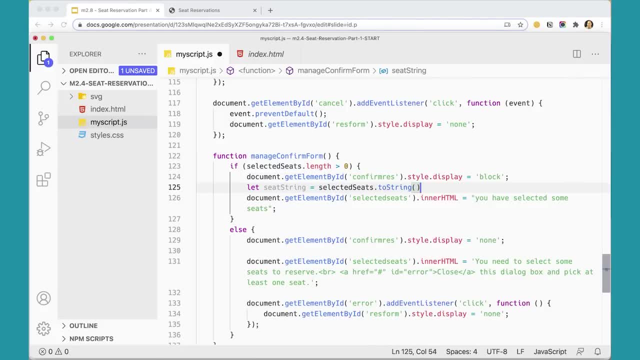 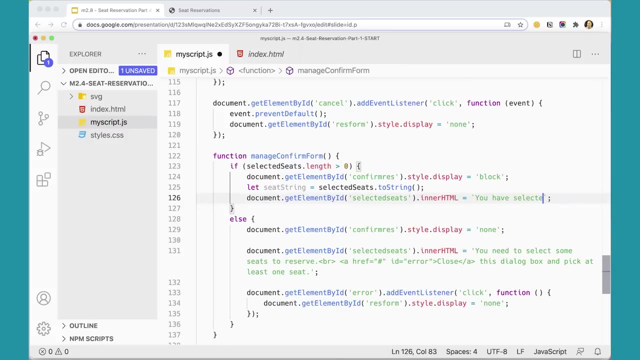 to string. so that's going to turn that into a string and then down here. this is now. now, since i'm going to put a variable in here, i need to use my tick marks- you have selected seats- and then i'm going to put in dollar sign- curly braces- seat string. 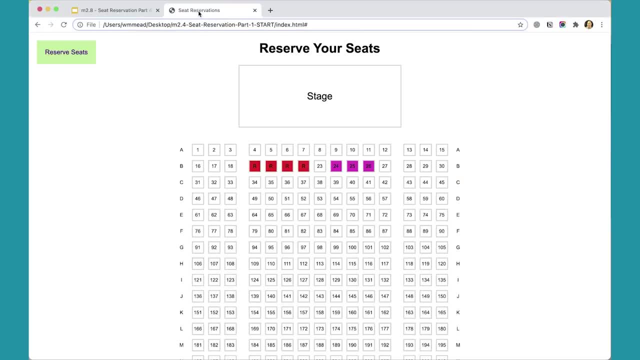 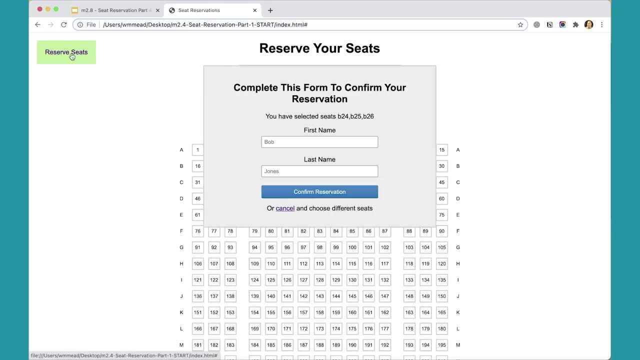 like. so let's see what that gives us if we come back here and click refresh, if i click some seats and click the reserve seats button, i now get this. so it's a little bit better. it still could be better because it's just, you know, we don't have a space after the comma. the last one could be: 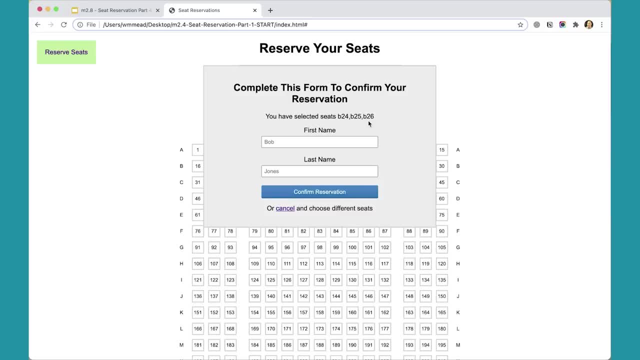 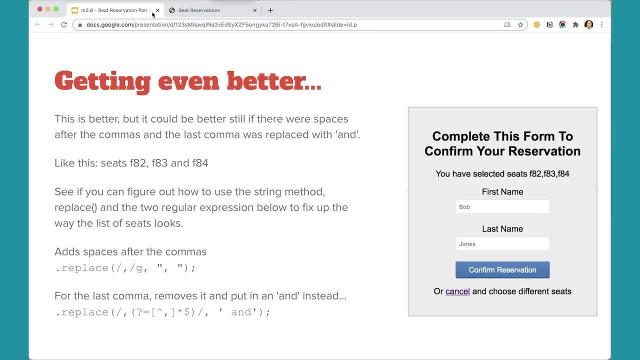 and so it says b24 comma, b25 and b26. that would be nicer, so we'll take a look at how to do that. next. here is your next micro challenge, we've we. what we really want are is something like this: f82 comma, f83 and f84. so see if you can figure out how to use the string method replace. 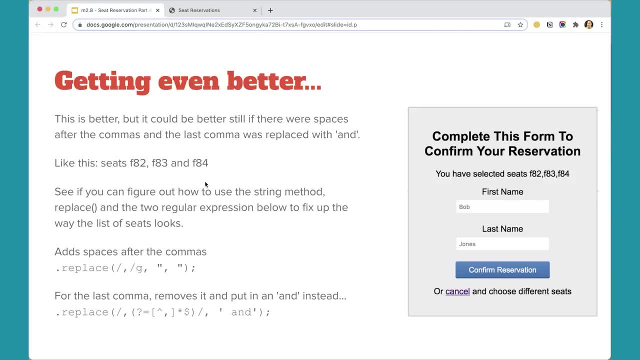 look it up on the mdn and see if you can figure out how to use it along with these two regular expressions which look a little bit funny. you'll have to pause this video and sort of type them out, but see if you can figure out how to use these two regular expressions that. 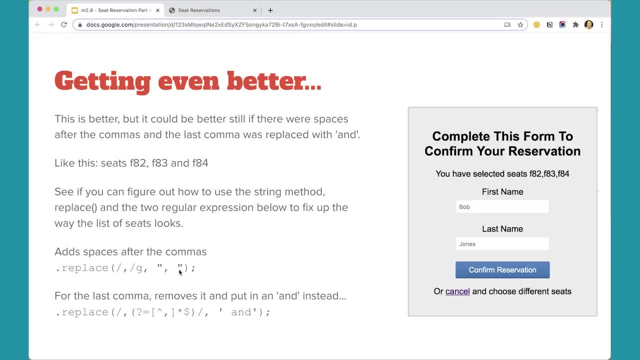 is this one here will add the commas and add a space after each comma, and then this one down here at the bottom: we'll put an and in in place of the last comma, a space and an and in place of the last comma to get us something that looks a little bit better. so see if you can do that. 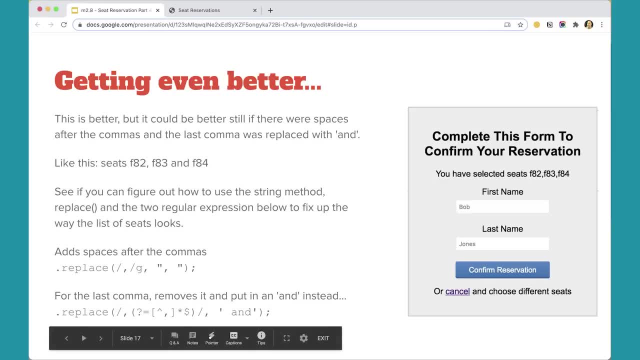 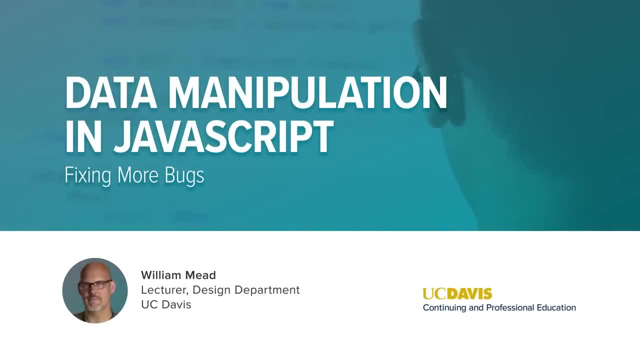 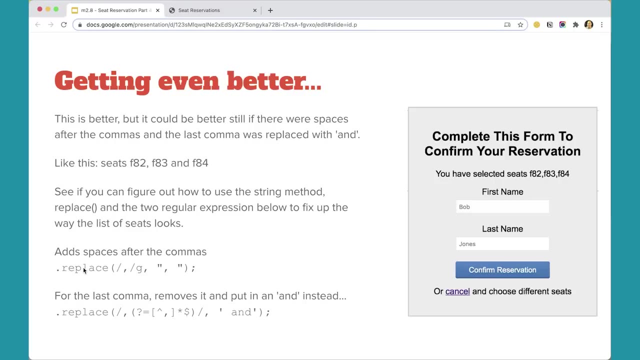 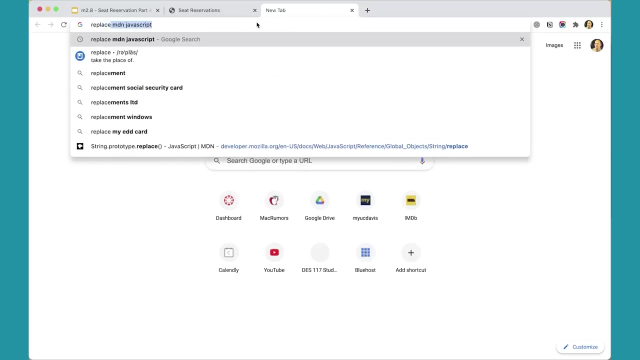 and then we'll look at the solution in the next video. were you able to complete this micro challenge? if you were, you should be able to use these, use the replace method here, and to find out about it, you can just go over and search: replace MDN. 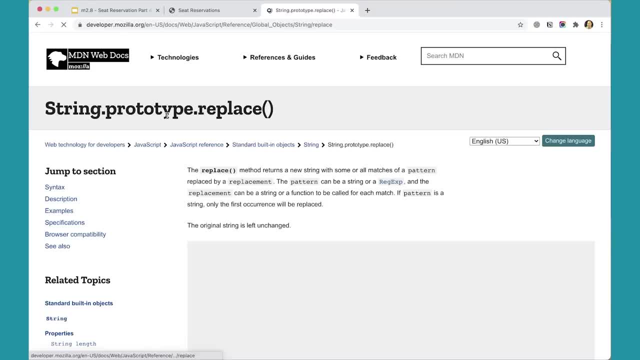 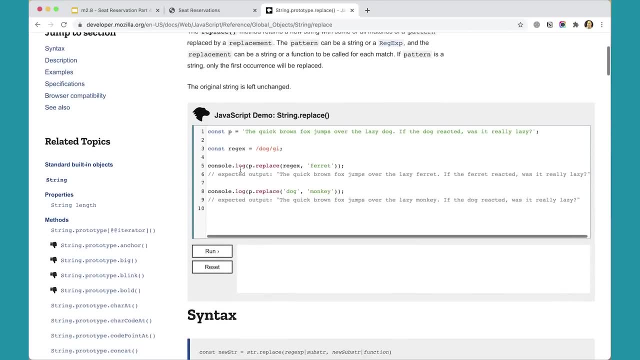 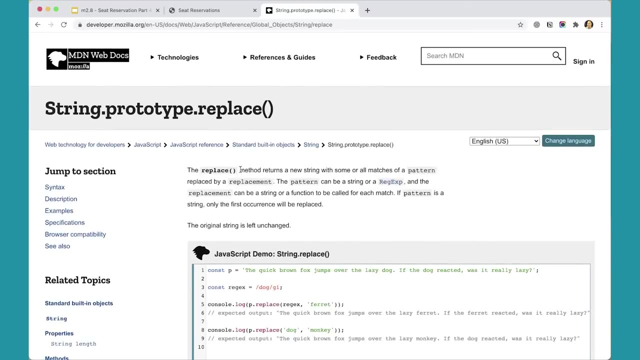 JavaScript, something like that, and that will bring up this page here, the string prototype replace page, which will tell you how to use this method, and it's really important, while you're working with JavaScript, to get used to using this documentation to see how different methods work that are built into JavaScript so you can use them correctly. so hopefully you came up with 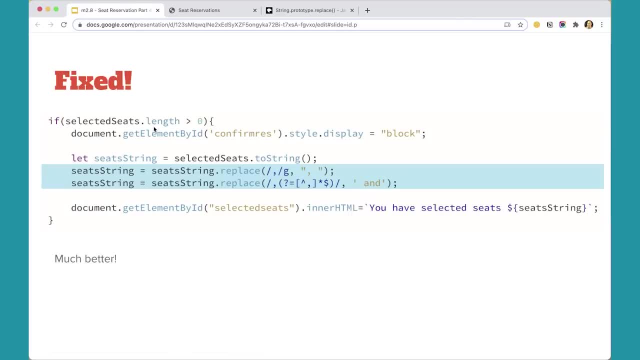 a solution that looks pretty much like this. so I've got seat string equals seat string. replace my picture here. I had an S in my variable here and mine. I actually don't have the S, so as long as the variables match, it doesn't really matter. I had seat string on mine, but I'm going to go. 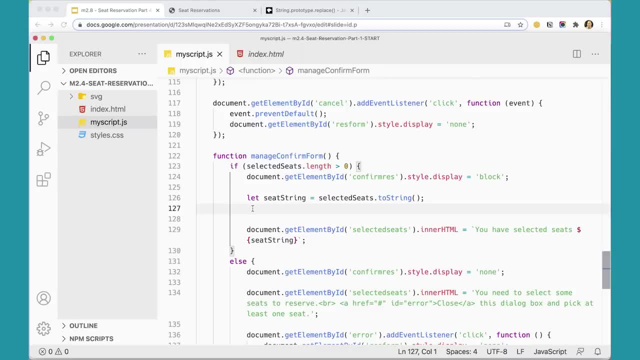 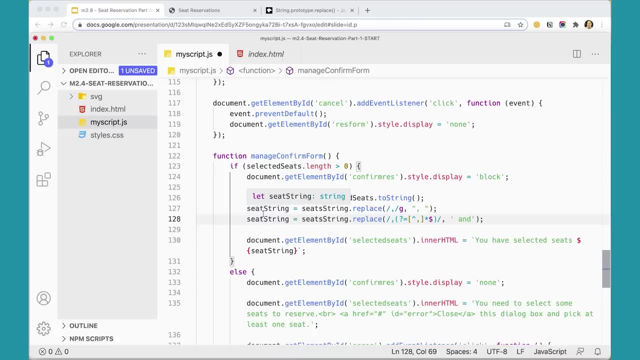 add this over here and I'm going to go add this over here and I'm going to go add this over here, over onto mine over here. I'm just going to paste it in so you don't have to watch me type it, but put this in and if you, if you're using, just make sure your variables match. I'm using seat string. 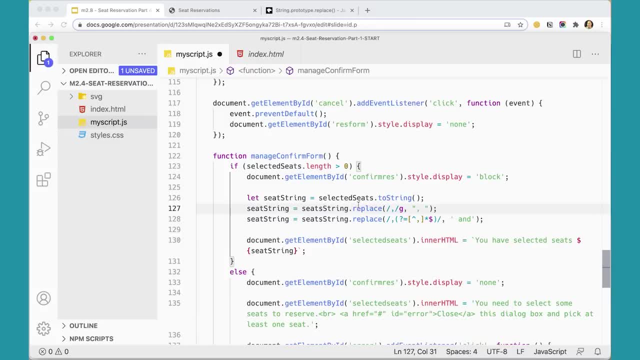 without the S here, but it's going to be equal to seat string replace and seat string replace here. there we go, so I'm going to replace those again without the S. it's got a little bit screwed up when I pasted in there. I have the S in there, so just make sure you get the variables right, because 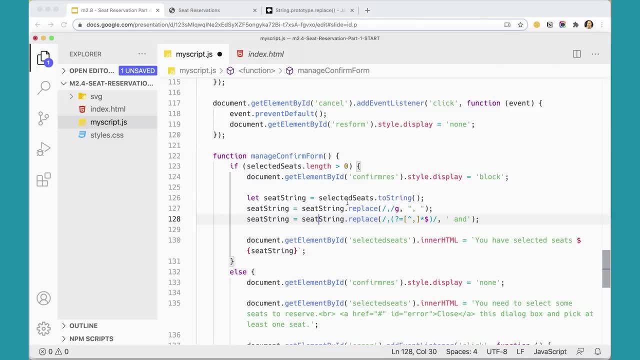 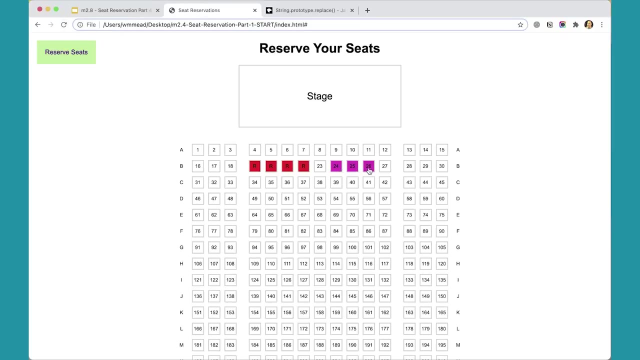 we're assigning back to the same variable the seat string with the replace method on it to replace those things down there as well. okay, great. so let's test this. if I come over here and refresh and click on some seats and click reserve seats, now I'm getting B24, B25 and B26, B26 and B27, so I'm getting the 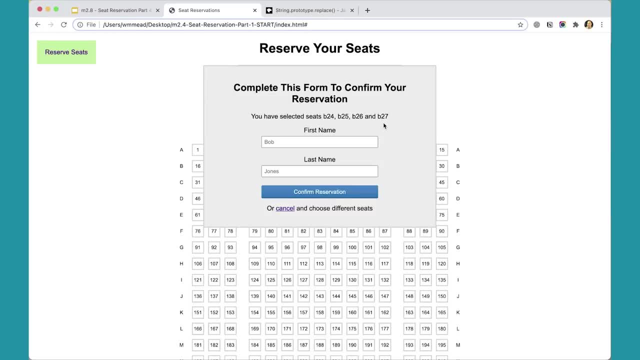 end, at the end there, and it's all looking much better. that's fantastic. I'm going to click cancel. now one last little problem here to fix: what if I just want one seat? I'm a loner, I'm going by myself, I'm going to social distance. 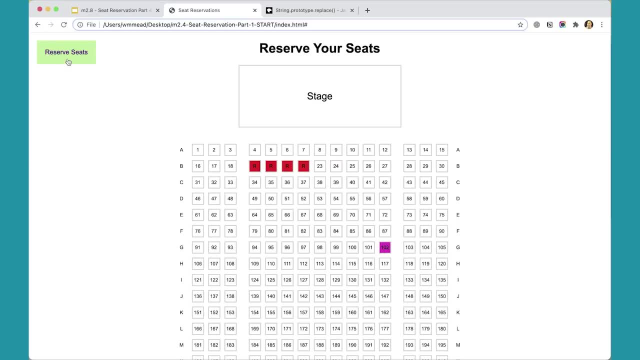 and stick myself down here away from everybody else, and I click reserve seats, this says you have selected seats G102. that doesn't make sense. why is the word seats here plural when I'm getting just one? this is a really minor thing, but language matters, and if we can catch these little issues and fix them in our code, I think it's even better. 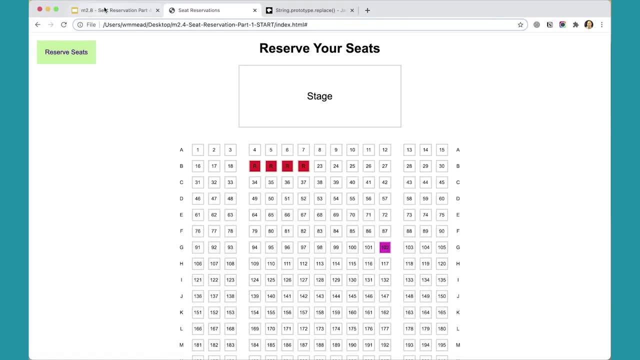 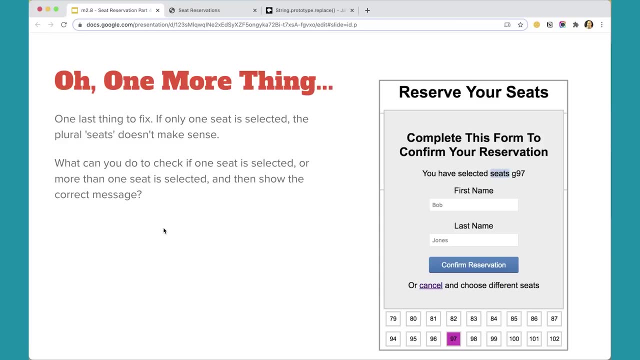 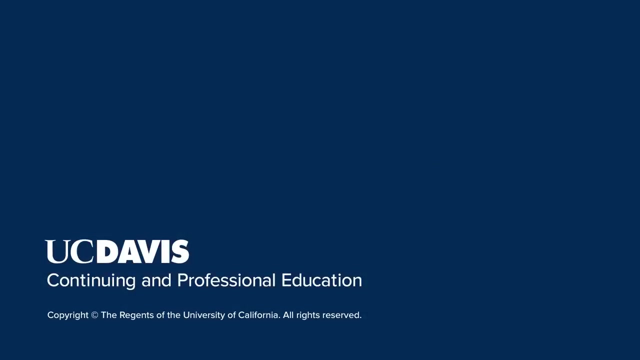 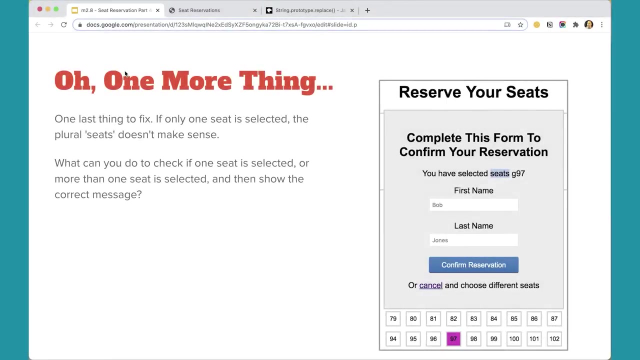 so our last little micro challenge here for this at the moment is to fix seats so that it's only if there's only one seat in the array we have, it'll just say seat instead of seats. so see if you can solve that one foreign. one more thing: were you able to solve this little problem here? hopefully you came up with an idea. 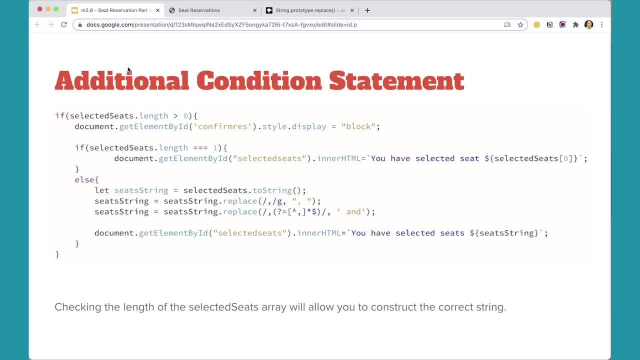 that looks kind of like this using an EFL statement. so if the selected seat length is exactly one, we're going to do one thing else. we're going to do the thing with the to string and the replace and all that stuff. so we're just adding one more, if else, statement. 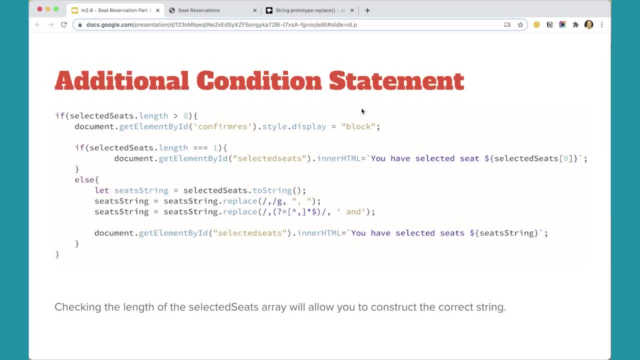 to kind of fix this thing, and down here you can see that i'm using just selected seats, square bracket zero. since there's only one element in there, i don't need to convert it into a string just to do that. so that was the solution i came up with, so let's go ahead and add this over into our. 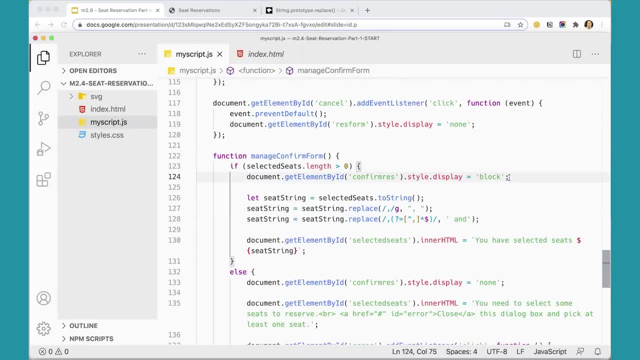 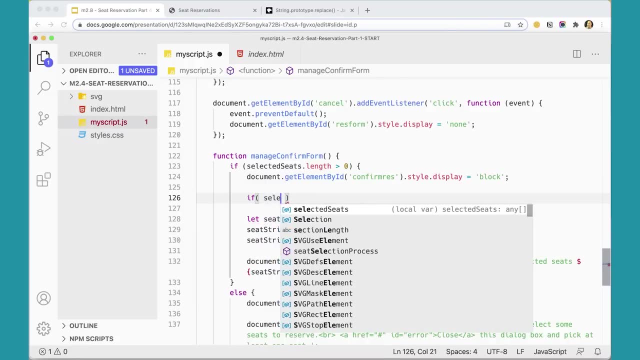 function over here. so that means in here. i'm just going to add an if statement here, if, and in there i'm going to check to see if selected seats dot length is exactly one. if it's exactly one, i'm going to do. i'm going to do one thing here. 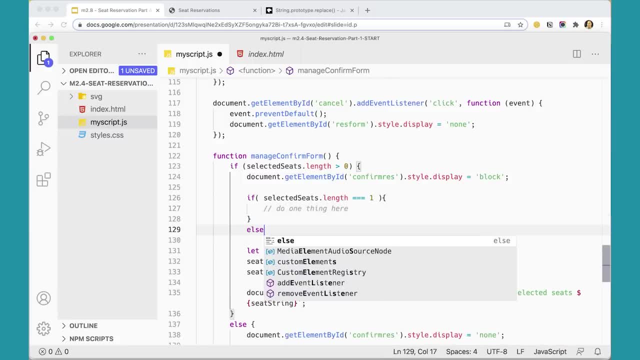 else i'm going to do this stuff and stick that in there, like so i don't need all this extra space. there we go. so what are we going to do in here? we're going to say document dot. get element by id, selected seats dot- inner html. 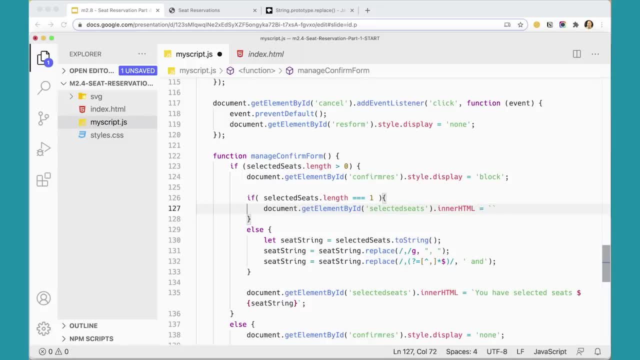 is going to equal tick marks. i'm going to use my tick marks because i'm going to have a variable in there. i'm going to say you have selected seat and then i'm going to use my dollar sign and curly braces to say whatever is in this array- selected seats. 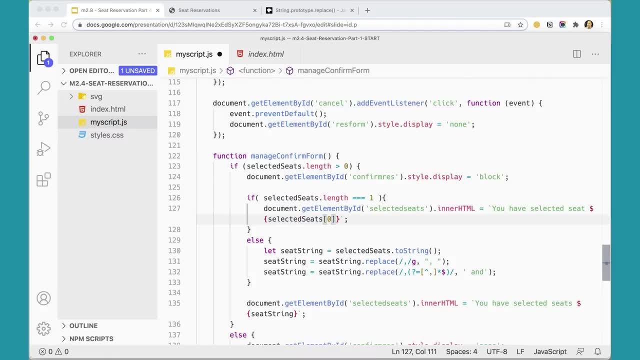 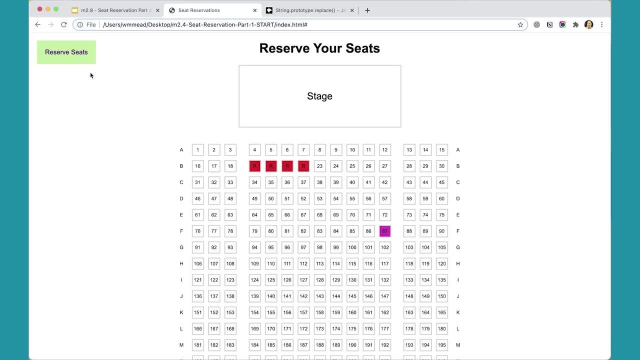 and because it's an array, you have to square bracket zero to get the first element in there. so now i've selected that one seat and put it in there. let's give that a try. if i come over here and refresh this now, i'm a loner going all by myself and i'm going to click a seat. 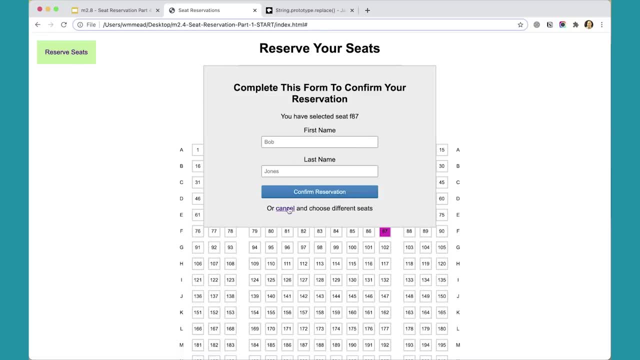 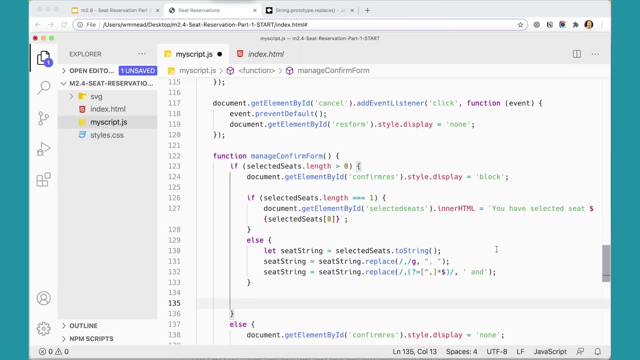 and it says: you've selected seat f87. if i decide no, i'm going to bring somebody with me and select seats now. oops, that's not working. what did i do wrong? i think i just need to move this so that it's inside the else. i think that's all i need. 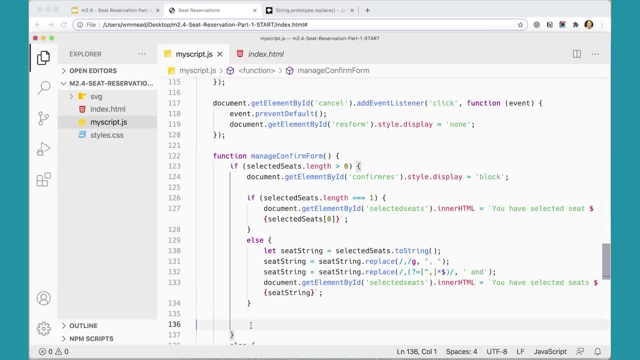 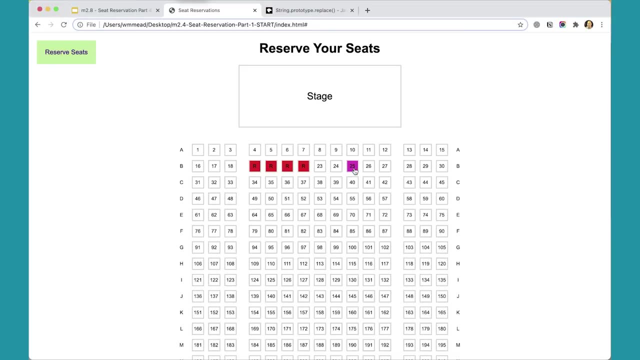 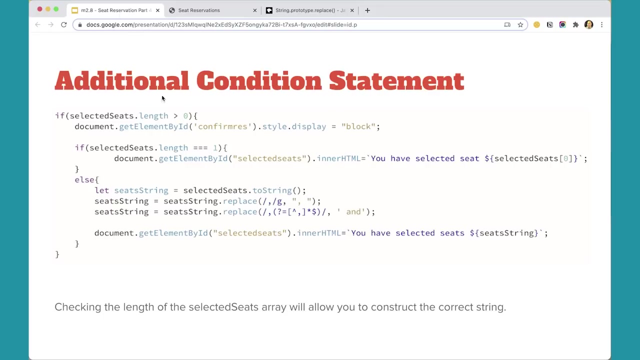 there we go, try that: select a couple seats, select a couple seats, and now i'm getting the correct thing- select one seat. and now i'm getting one seat, okay, great, so that's all working really well. and, um, we've got all those pieces in there. hopefully you came up with this same solution here and you can. 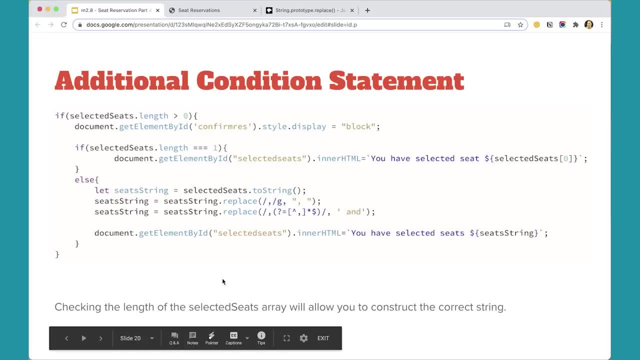 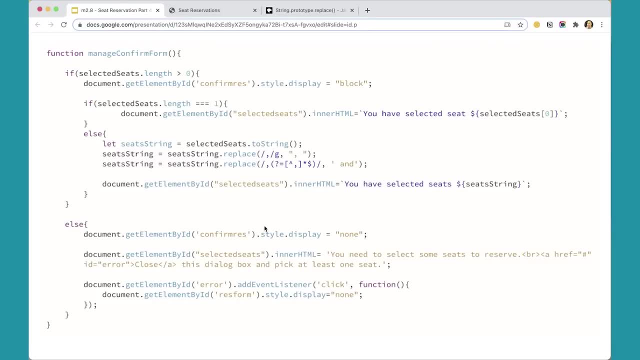 see, i forgot to put that in that else statement. okay, great, so that's working really well. here is the full function and it's a long function. there's a lot of stuff going on in this function but it's not really difficult things. we're just using basic javascript to manipulate the html. 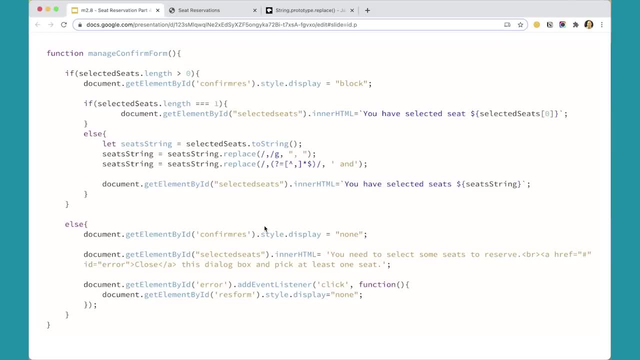 that's going to go on in that form and whether or not the form is going to display or what part of the form is going to display, based on what users have selected. and that's sort of the moral of this particular part of this project. is that thinking. 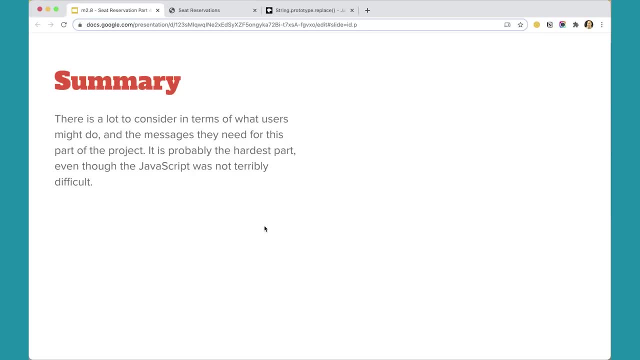 about what users could do and where things could go wrong is probably the hardest part of any interactive project like this and um, usually if you're fixing bugs, it's in finding new ways that users can screw up and mess up your product, mess up the process of completing a task in a project. 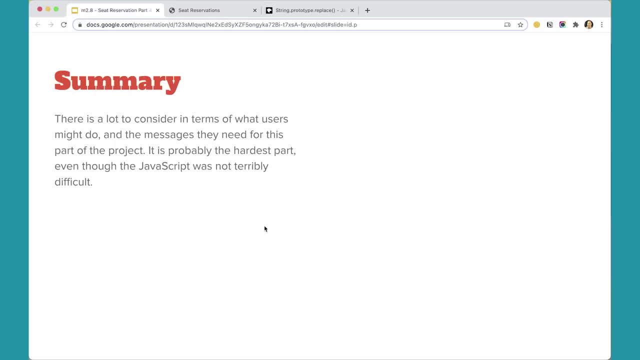 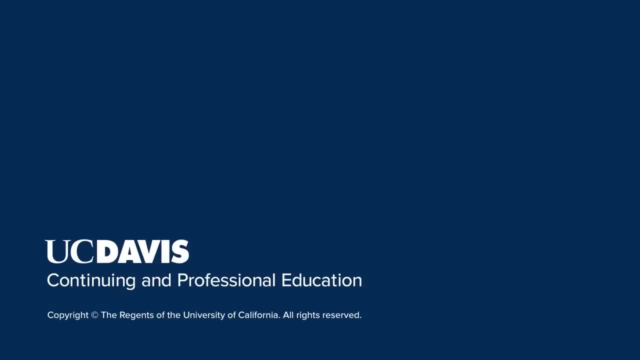 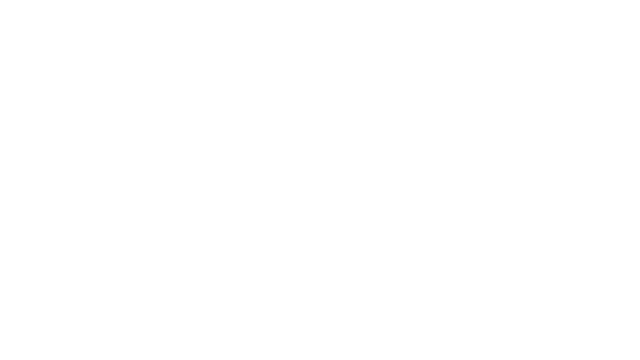 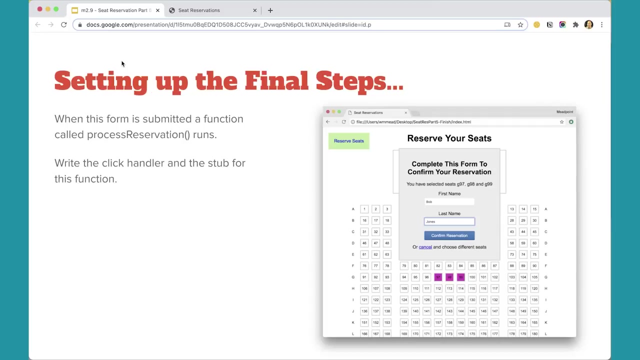 and if you can sort of route those out, figure them out and then solve them, your project will get better and better over time. seat reservation program. part five: reserving the seats. so these are really the final steps that we need to do. we've done a lot with this. 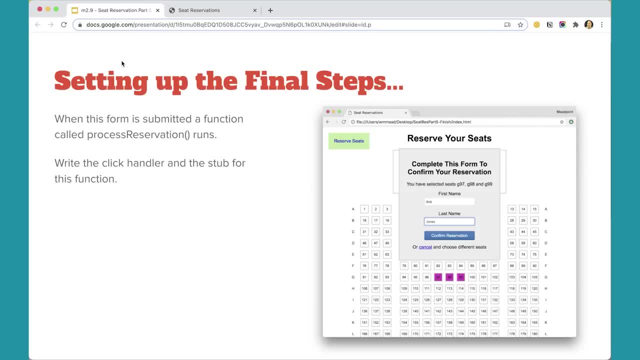 project and it's a long project. there's a lot of pieces to it, but the final part that we need to figure out is how to, once a user has put in their name and click that confirm reservation button, how do we take the seats that they've? 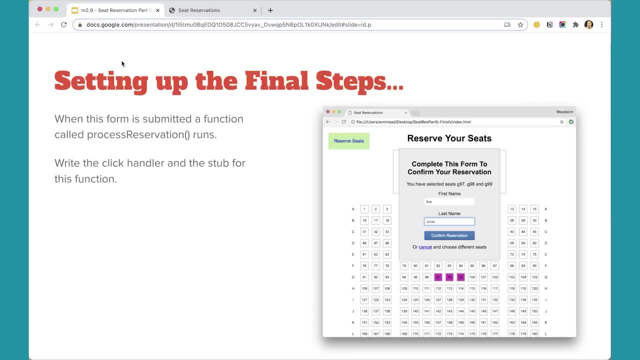 selected and put them back into the object, the- the reserved seats object- up at the top of our javascript file, which would simulate putting it back to the database, perhaps. so, um, that's kind of what we need to do next. so what we need to do is write a click handler and create a function. 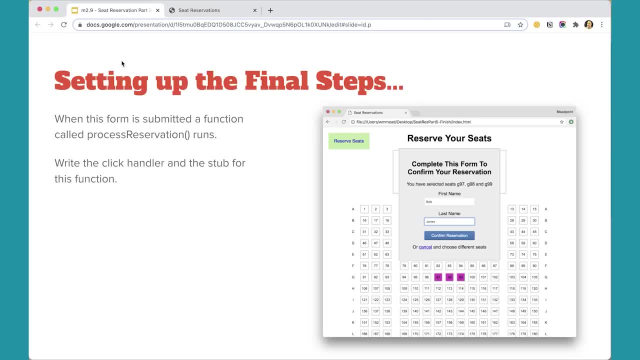 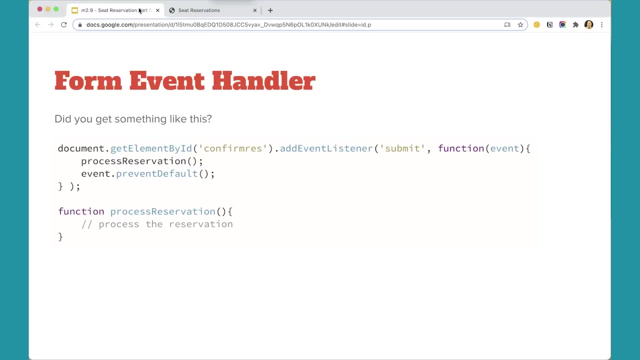 called process reservation. that's going to run when the click handler is clicked. so let's do that first. see if you can do that without going forward in this, uh, in this video. pause the video and see if you can do that part by yourself. did you get something like this? i have an event handler looking for the submit button on that form. 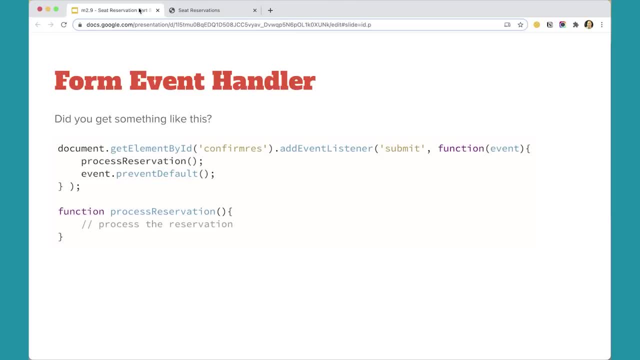 for the submission of that form and when it's submitted i'm going to prevent default because i don't want the form to actually get processed, i don't want it to go off to a processor or anything like that, but i want to capture that submit event and run this process. reservation. 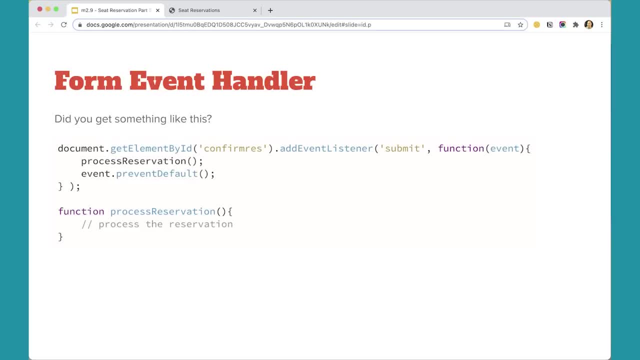 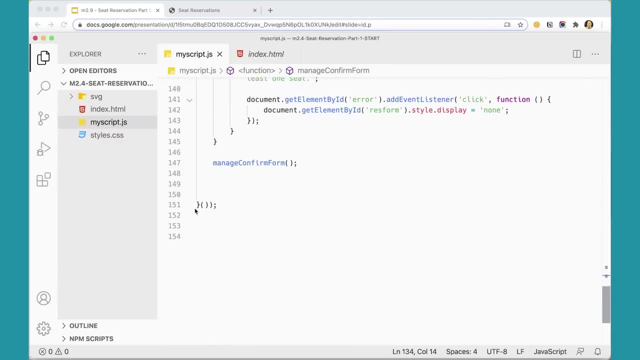 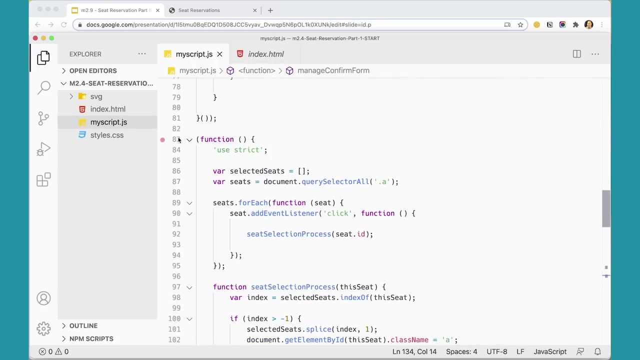 function. so let's go ahead and add this over into our event handler and see if we can do that file over here. in case you got lost or stuck, i'm going to stick it inside of this iife immediately invoked function here that i have up here in line 83 on mine. 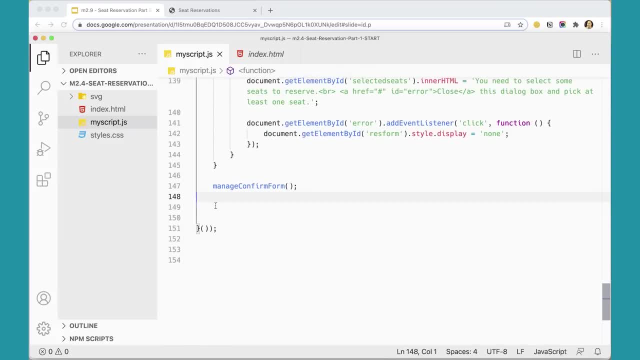 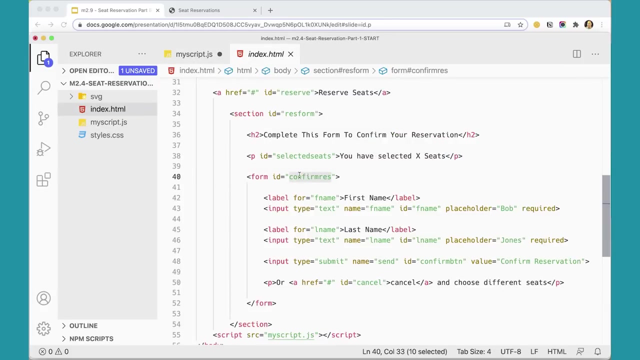 this immediately invoked function expression, this closure. i'm going to just stick it in there again, just keeping everything inside of closure. so i'm going to just put a document type: get element by iu white house blink Friday out current form CHI 123. so i'm going to show you some which are original form: red box: 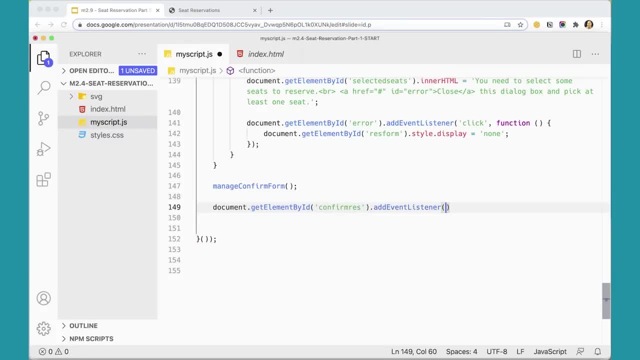 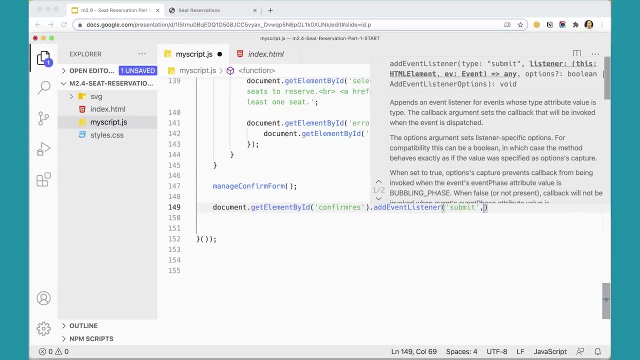 over here. you can just take out the periods side and look at this your and click here. so i'm себе, um, and of course we are going to speed things up for this add a function and that actually works quite well. we're going to go ahead and send this information and look. 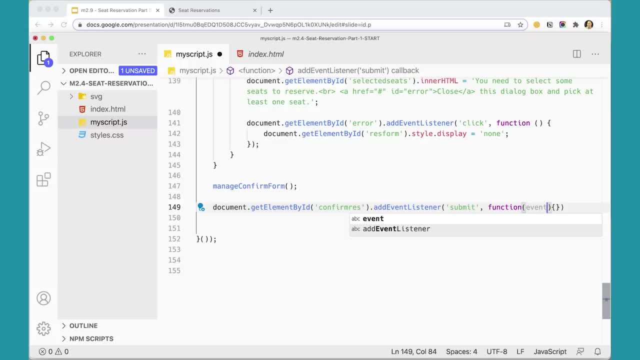 right here we're going to pass in the event, like so I'm going to put a semicolon at the end of the line and then inside the curly braces we're going to do eventpreventDefault. And again on my picture a minute ago: 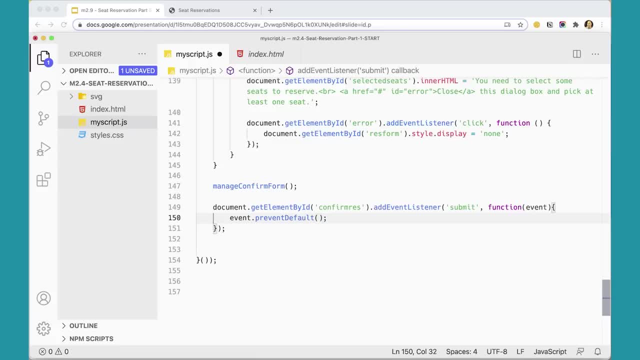 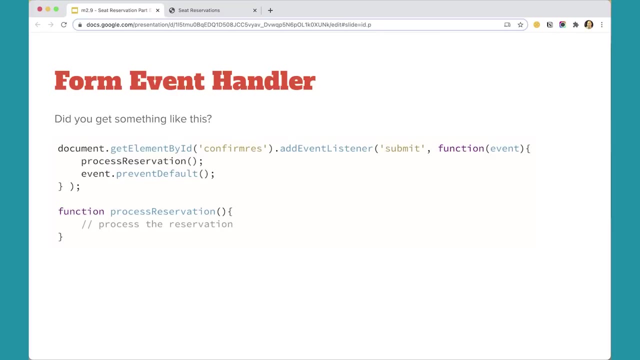 you saw, I put that at the bottom. It doesn't matter if it's at the top or the bottom. We're going to preventDefault. but then we're going to run a function called- and what did I call it again- ProcessReservation. just want to match what I have here. 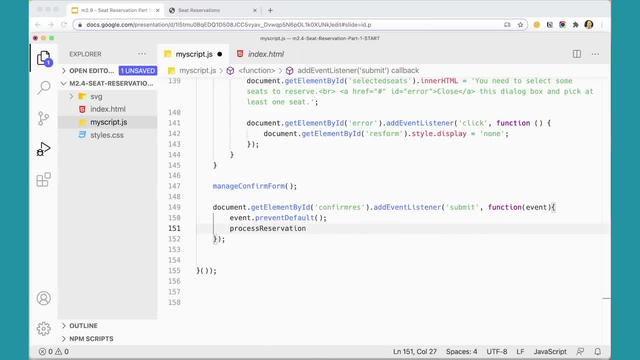 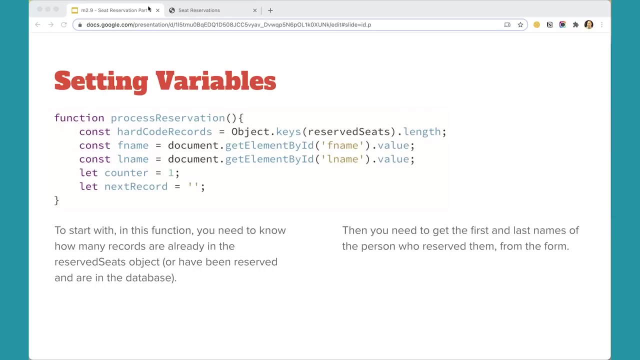 ProcessReservation. we're going to run that function, So down here now I need that function- FunctionProcessReservation- there we go. So I've got that stubbed out and ready to go. Hopefully you got something similar At the top of this process- reservations function. 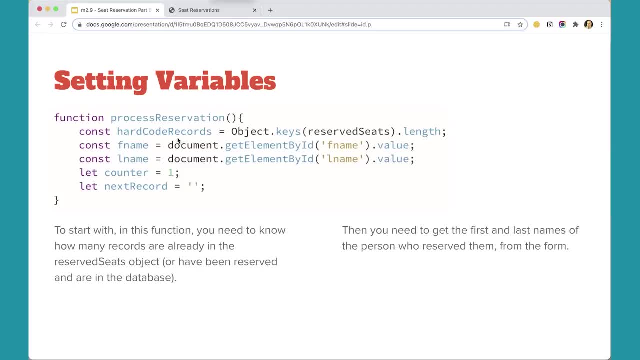 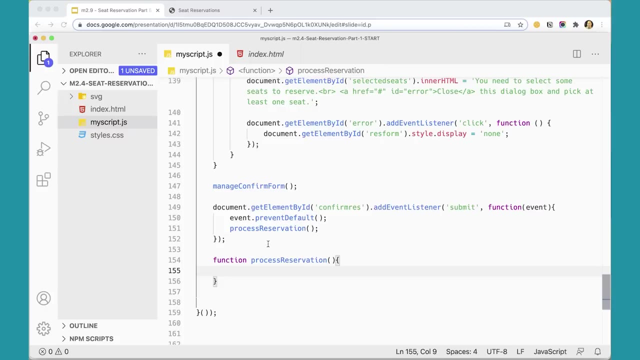 we need some variables. First, I need to find out how many records are in the reserved object to begin with, So I want to count them up in this object. keyslength will give me that information, So I'm going to add that in over here. 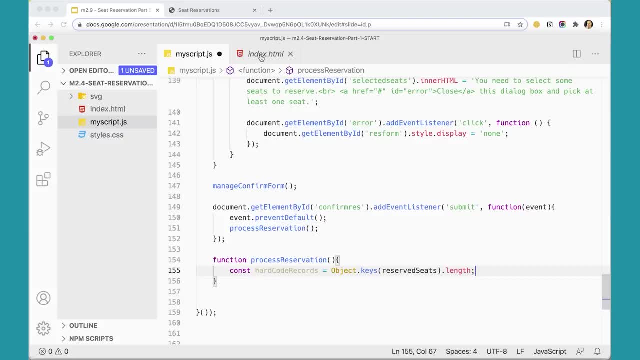 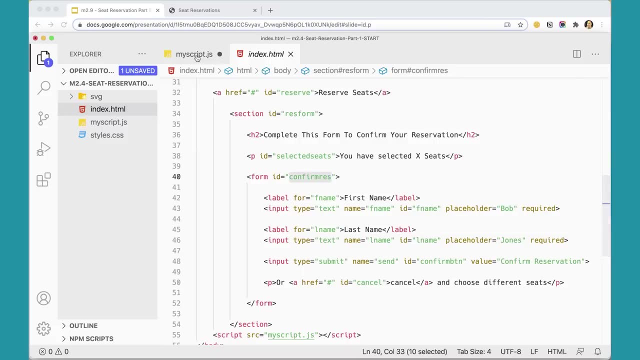 And then the next thing I need is I need to get the value that somebody has typed into this form for the first name. So I need the value for the first name and the value for the last name, So I need those as well. So I'm going to have const. fname equals documentgetElementById. 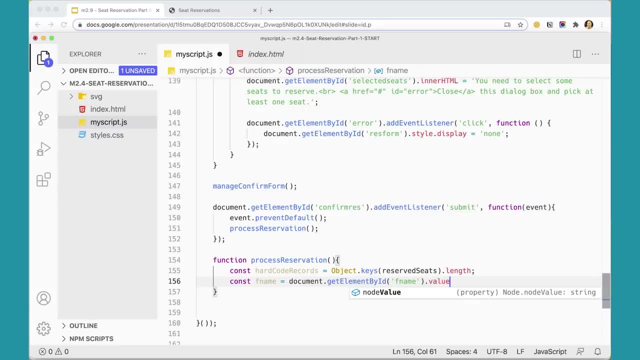 fnamevalue. so I need that one. Whoops, Not no value value. And then the same thing for the last name. So that's going to be lName and this one's going to be lNamevalue, And then I need to counter. 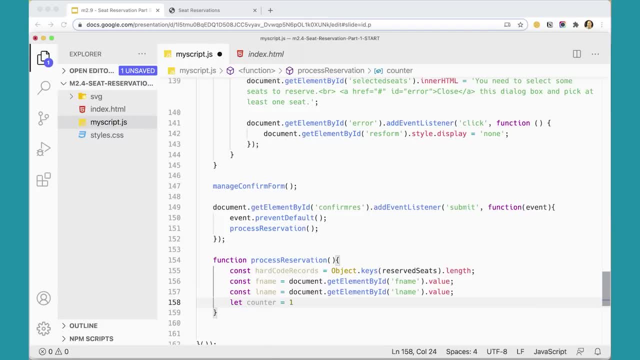 let counter equal one, And I'm using let here because the counter is going to change As we go through stuff. you'll see what we'll do with that for in a minute, And then the last one I need is just an empty string. 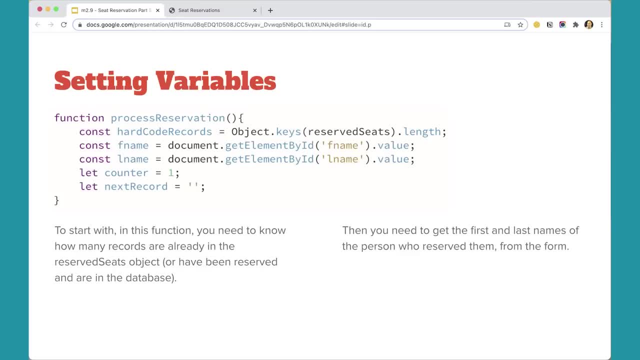 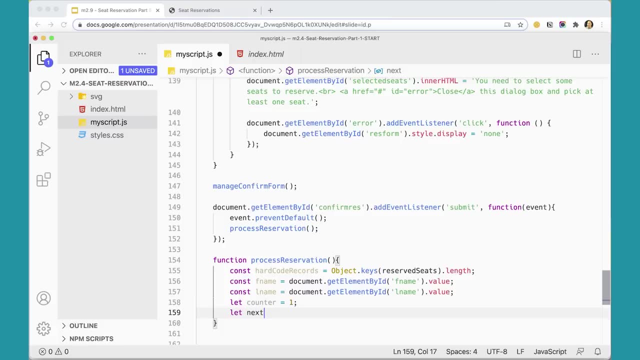 for next record, and we'll fill that in as well. So let's add that as well. Let next record equal one Quote. quote for right now, We'll just leave it there, Okay, So we've got some basic variables to get started with. 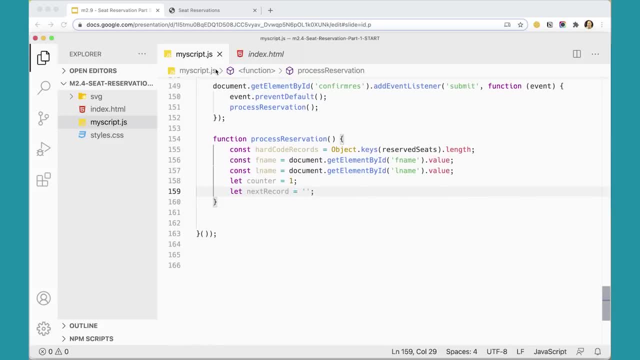 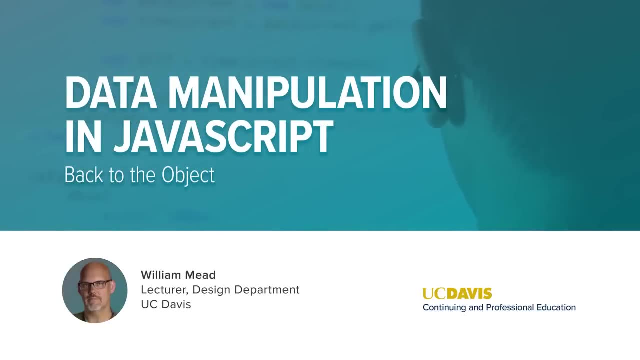 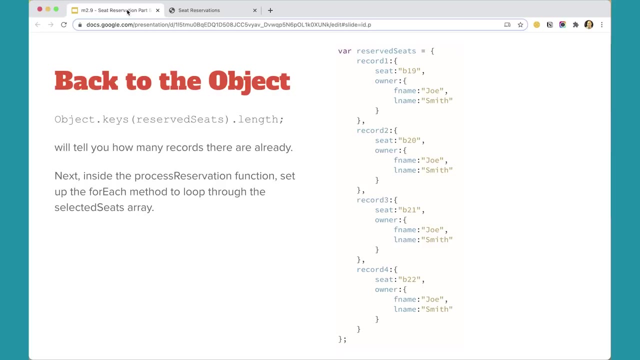 and then we'll pick up filling out this function further in the next video. Okay, So again, the objectkeysReserveSeatslength will tell us how many records we have records we have in here for currently. that's what was built into that object to begin with. you could. 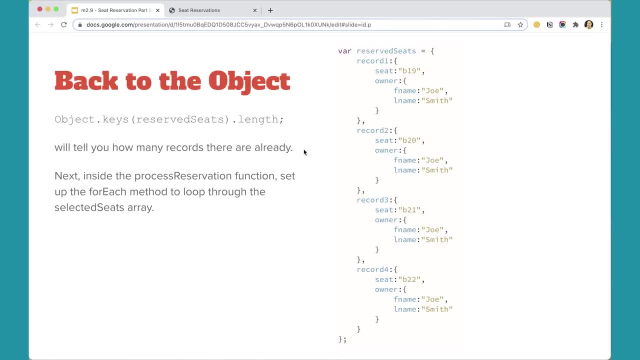 add more or take some away or something like that, if you wanted to just have to hard code them in. so we've got that. but next, inside the process reservation function, we need to use the for each method to loop through the selected seats array, because we're going to do a bunch of 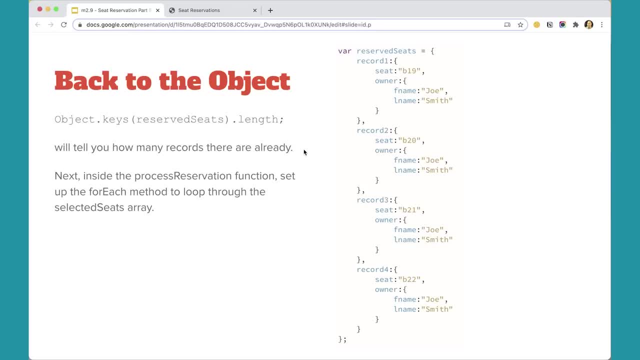 things with those select, with each of those selected seats. so here's your. your micro challenge for this point is to just set up the for each loop for the selected seats array. so pause the video here and see if you can do that without looking at the next part of the video. 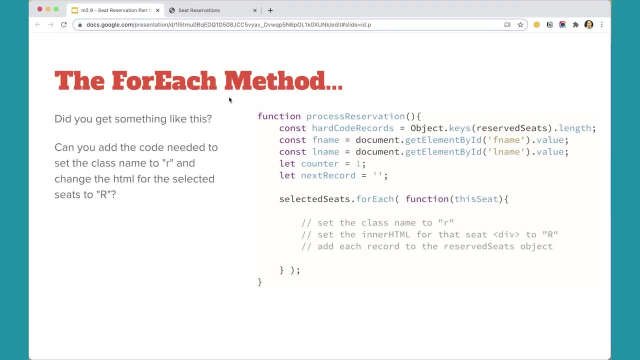 did you get something like this, the selected seats array you can see down here at the bottom. so we're going to go through selected seats and do something for this seat or for each seat in the selected seats array that has the seats that have been selected by the user. 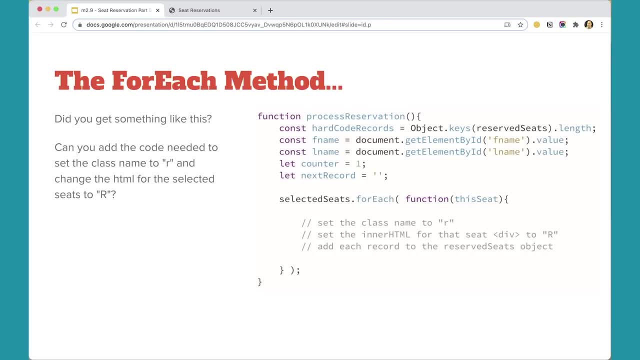 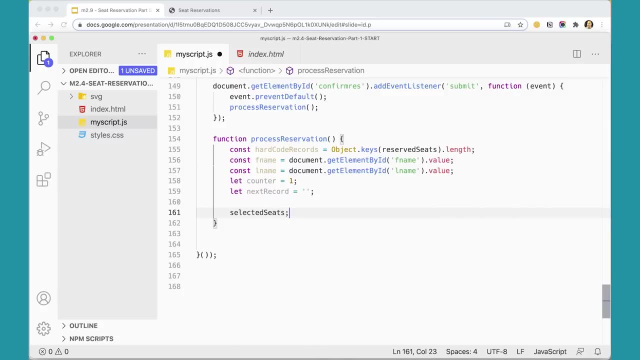 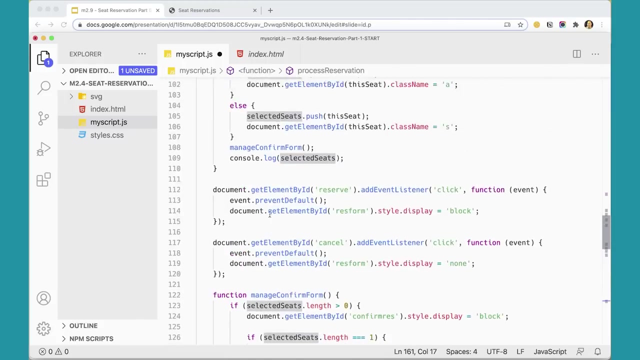 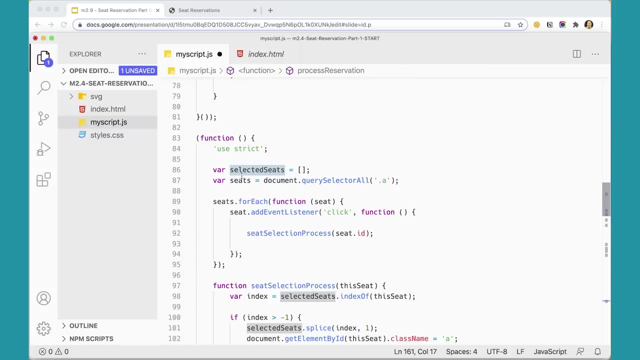 so let's go ahead and add this over there if we want to get this set up. so in here i'm going to say selected seats, dot for each, and we have access to this selected seats array because it's inside the, the um, the, the closure here, but it's at sort of this top level, so we have access to selected. 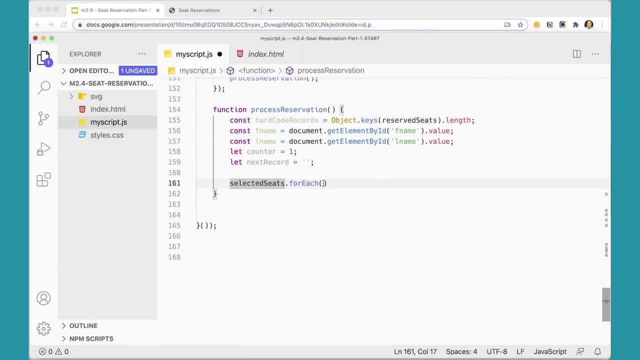 seats here, so we can just do selected seats for each and then in for each, put a semicolon there, in for each. we're going to do a function like so and we're going to pass in this seat and we're all set to do some things here. now, one thing we want to do for this selected seat: 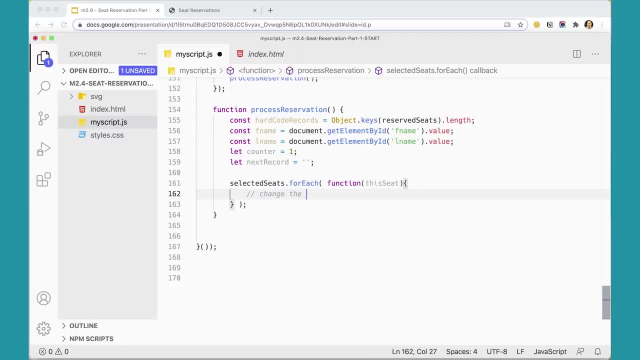 is, we want to change the class from s to r, we need to change the html to r and we need to add it to the object. those are some things that we need to do inside of this for each, for each seat that's in that array. can you handle the first two parts, this part in this part? 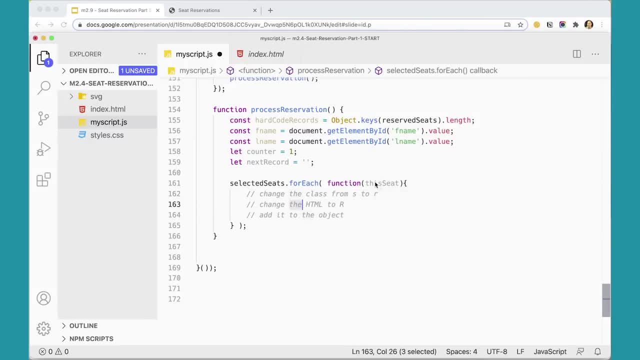 you should be able to remember. this seat is each seat in the array, so that's the id for each seat. so you just need to set that over. so see if you can do that. i'm going to do it here, but you can pause the video before i do it. 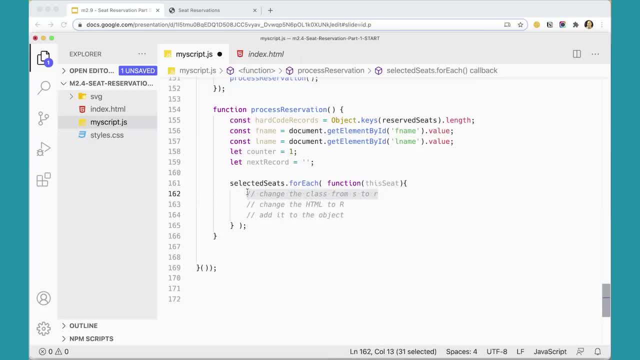 and see if you can do it for yourself. so i need to change its class. so i'm going to do document dot, get element by id. this seat dot. class name equals quote r. and then we need to change the inner html as well. so i'm just going to copy this: 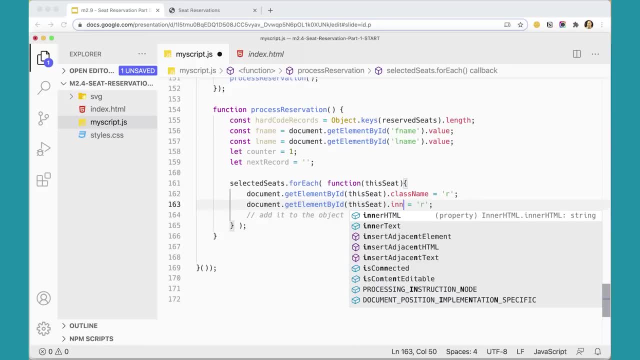 get element by id, this name- and i want to change inner html. i'm going to make it a capital r. hopefully you got that. that's not too hard, but i'm going to do it hard. we've done that before, okay, so that shouldn't be too difficult. to micro challenge now down here. 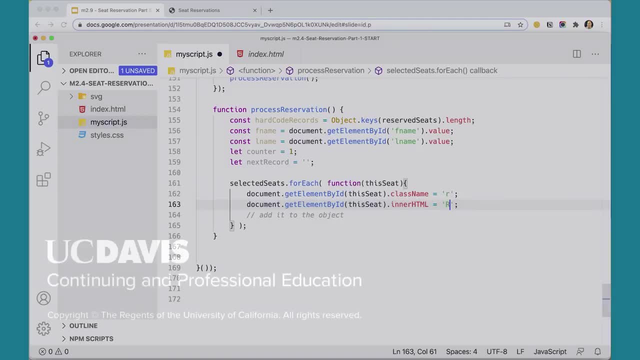 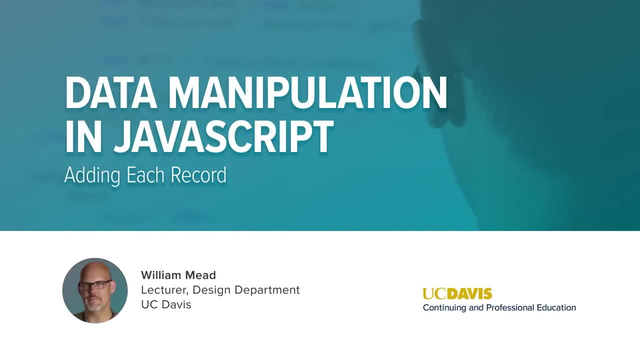 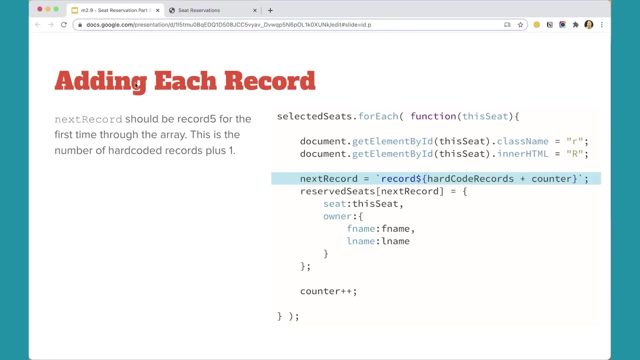 we're going to add it to the object and that's where the new bit comes in. okay, so now we need to add to our object up there at the top of the page and, if you remember, if we go back and look at our object really quickly up here, 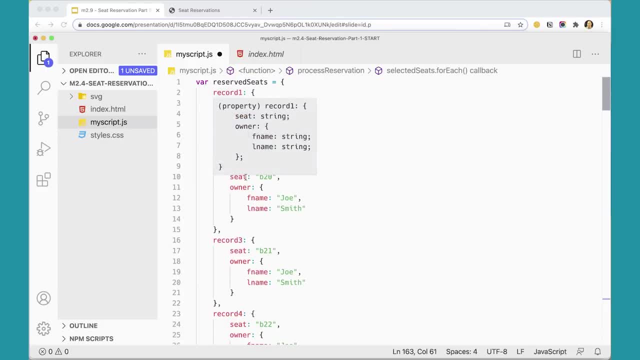 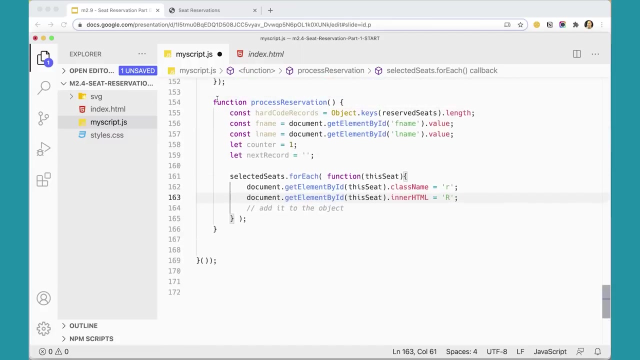 each record in the object starts. we've got record one, record two records be record four. so we need to add the next one will be called record five. it's going to be a number, the word record and a number five, and so we can do that down here by very cleverly coming in here and 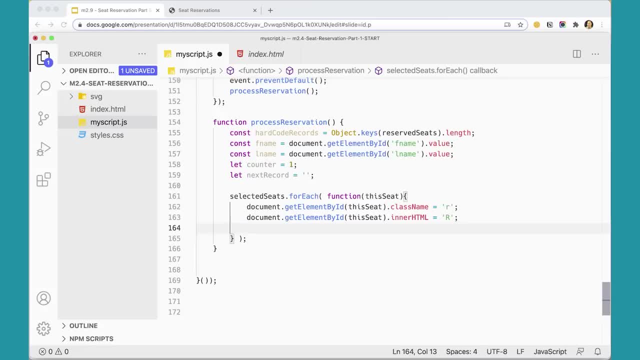 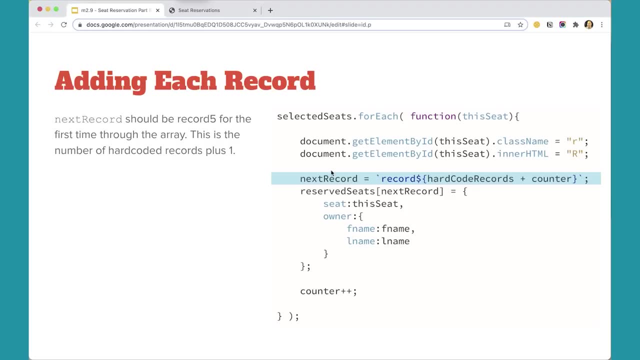 saying using our variables that we created up here to do this. so now i'm going to add, i'm going to change that next record variable so that it has the word record, and then i'm going to take the hard-coded records, which we know is four, because that counted those. 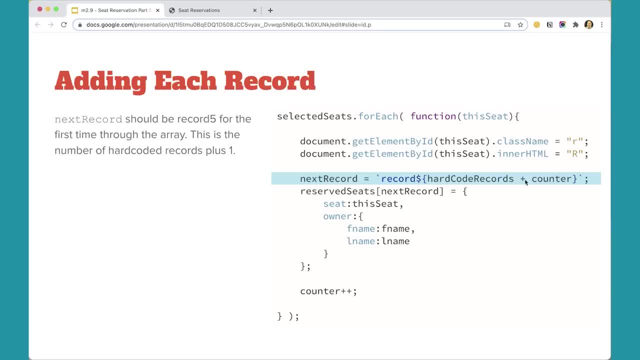 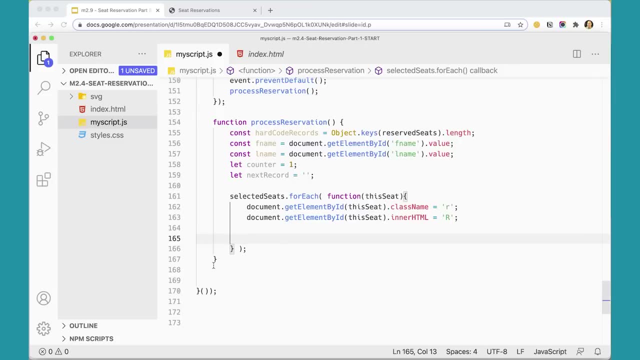 and we're going to add the counter which started with one. so that's going to make it a five. so this is going to be record five here. that's what that's going to say. so let's go ahead and add this in over here. next record equals- and i'm going to use my tick marks- the word record. 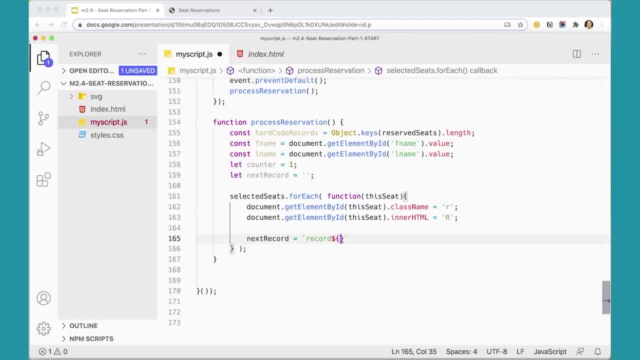 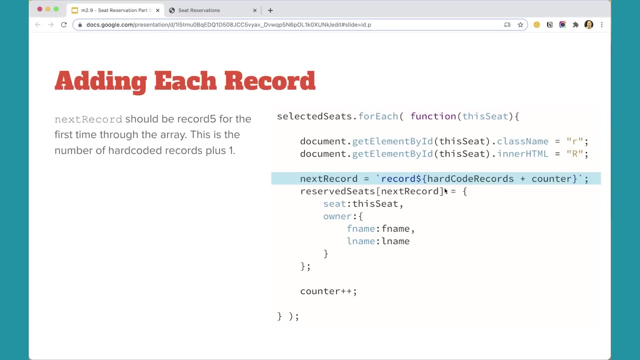 and then dollar sign, curly braces, hard-coded records plus the counter, which is one. so that's going to get me a five. so that's going to put that into next record. great, so now. now i need to actually add my object over here. so reserve seat, square bracket. next record. 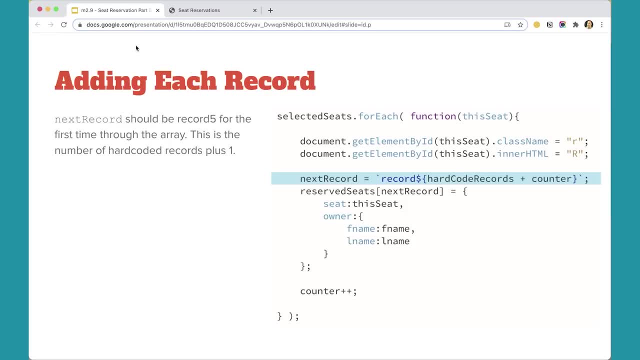 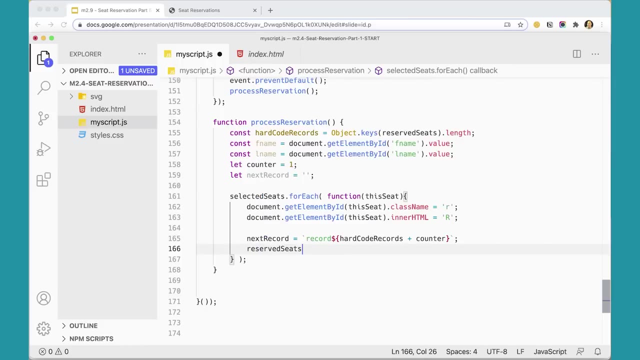 and then it's going to be. i'm going to use my curly braces to create this object or the, this additional element to the object, to the reserve seats object. we're adding to that to the object that already exists. so over here, reserve seats, square bracket. next record which: 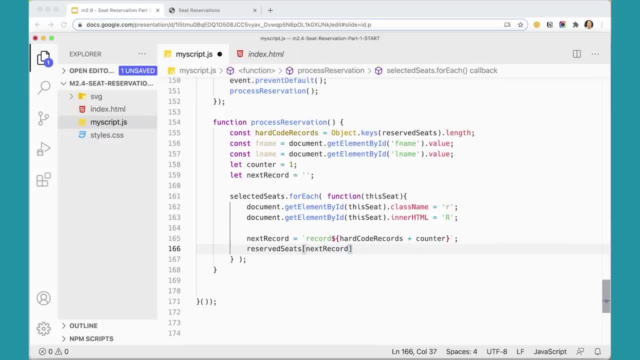 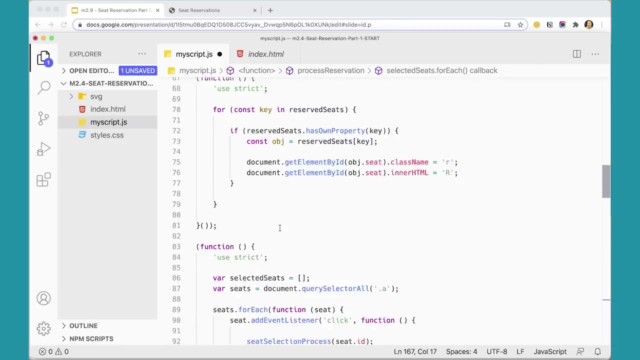 we know will be the word record and a five for the first time around. um, that'll be a five. so it'll say: record five equals curly braces. and then what are we going to put in here? well, we need to sort of keep working on the same structure we have here. so i need the seat. 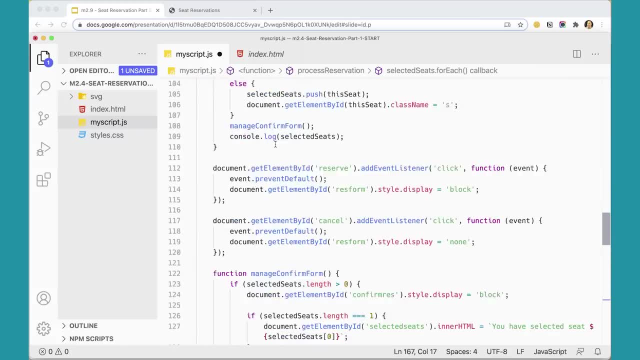 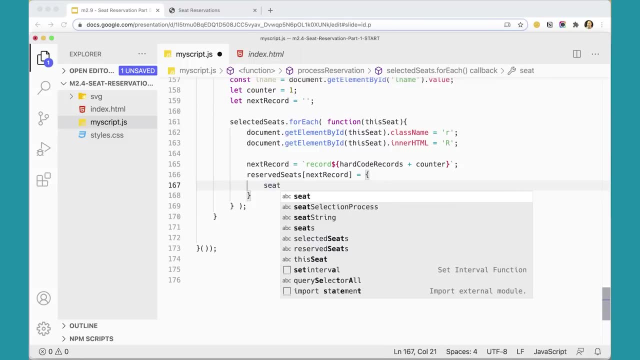 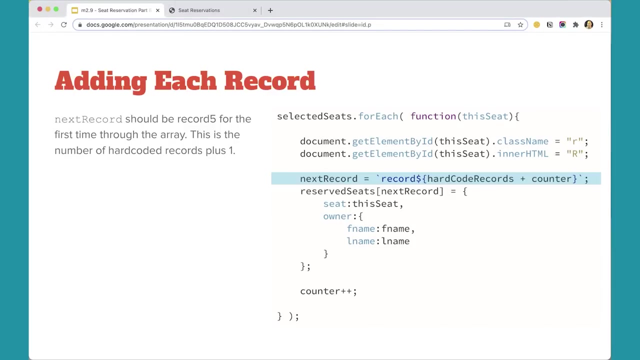 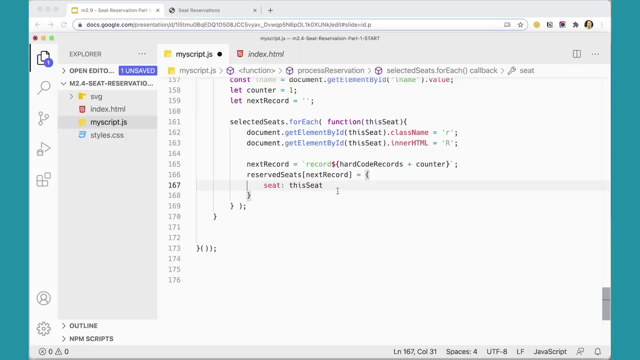 and the seat number and then i need the owner with the owner name. so down here i'm going to add seat colon and the value of the seat, which is this seat. right, that makes sense the seat, because that got passed in here. so we're adding that. and then we need to add another object. 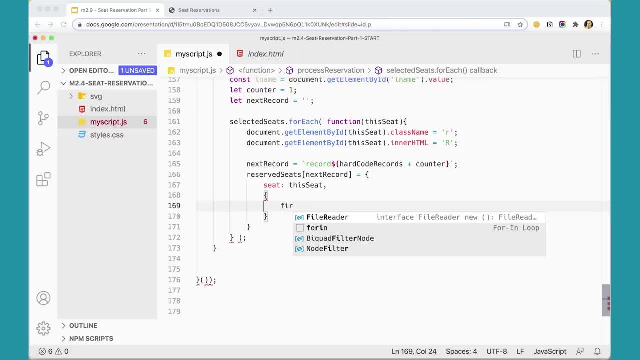 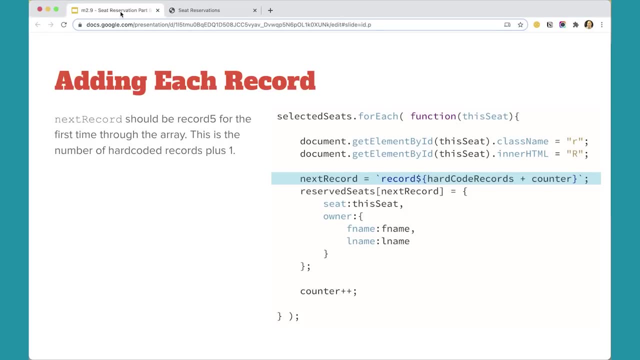 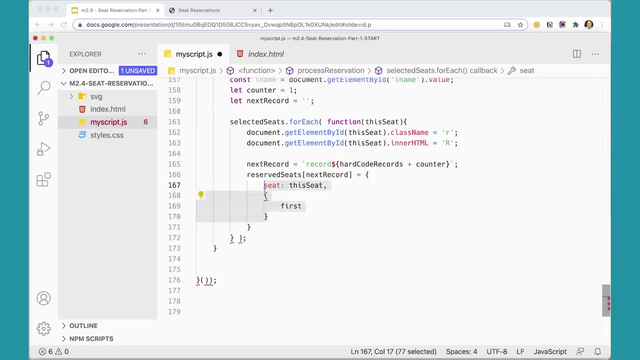 and this object is going to consist of first name. what did i call it actually? i called it owner. i did that wrong, fix that. and owner and that's an object that has f name, which is going to be f name, that variable up there. so we created f name. 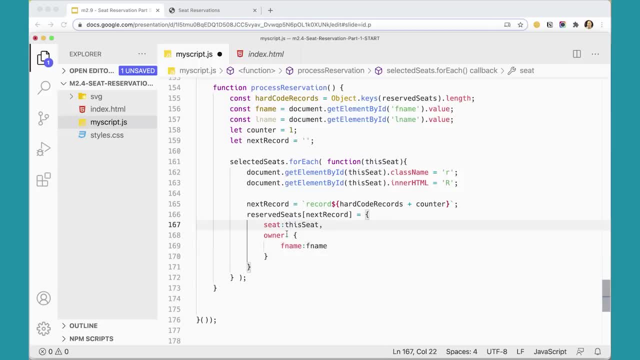 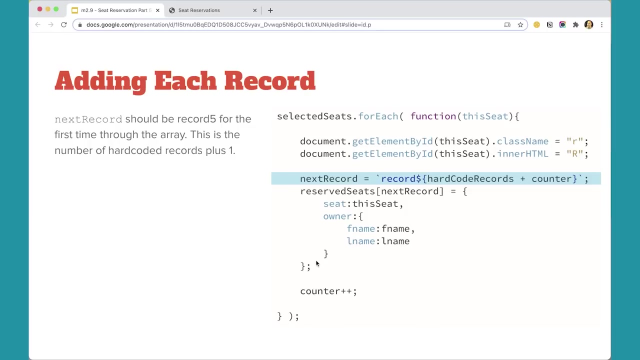 i think, spaces direction, then a comma only, which is only so that's going to set those variables for this record, number five. so that puts those in and that's great, and then all we need to do is increment the counter so that for each seat the counter gets. 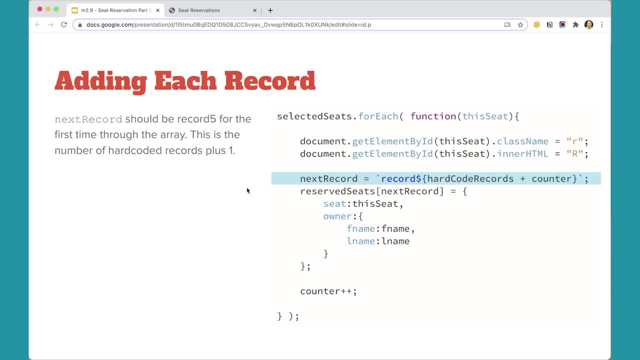 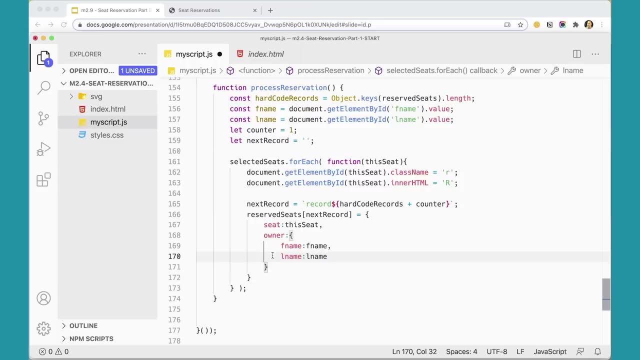 incremented up and incremented into the correct place. so for the next record in the in the array. so, after this thing has been all built, I'm going to do counter plus, plus and that should put them into the object. and look, this thing added the spaces back in. listen, as I saved it. that's fine, okay, great, I think. 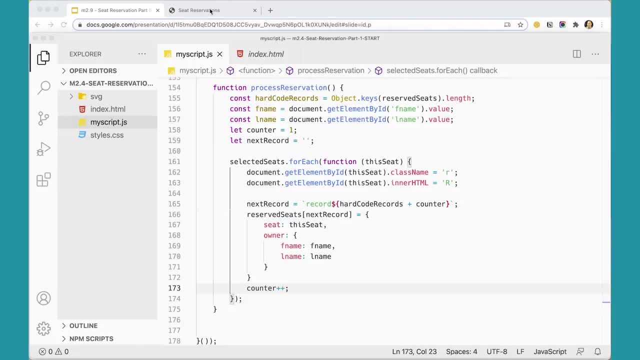 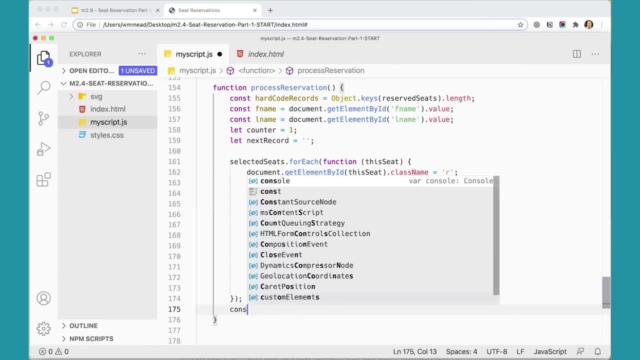 that should work. let's test it over here. actually, before I test it down here, I'm going to just do a console log that shows reserved seats so we can see that they're actually going in there when this process reservation happens. so let's see if that works. 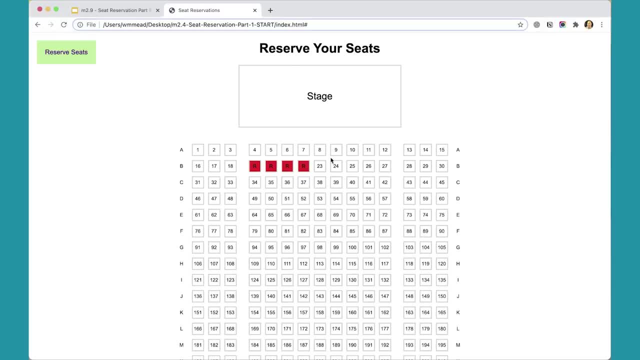 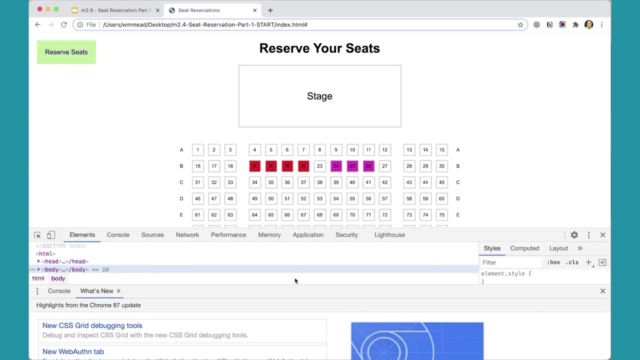 I'm going to come over here and refresh the page and now if I click some seats turns on the inspector here so I can see what happens. press the bottom of the page. I'm getting these arrays because I've clicked these seats. I have another console log in there. 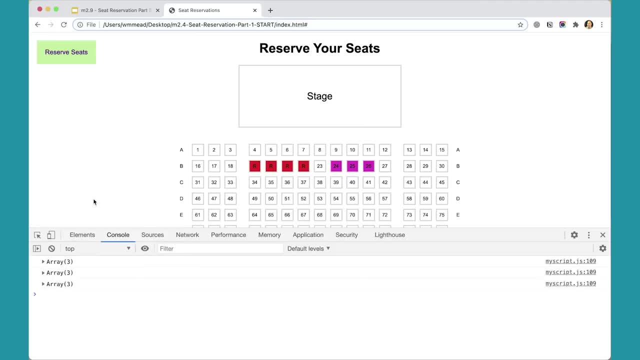 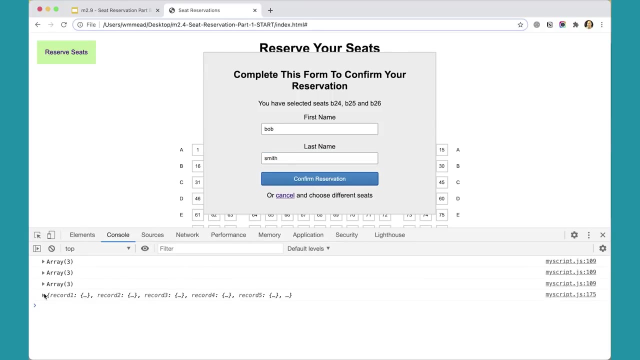 you remember, but it's okay. so If I click reserve seats and put in Bob Smith or whatever name you want and click confirm reservation, you can see now I have all of these additional records in here with the owner Bob Smith and seat B24 for each of these new records. 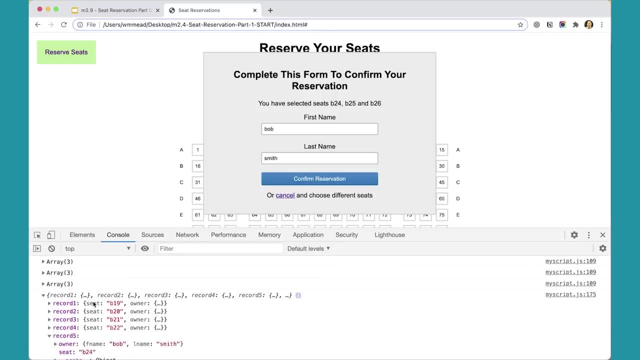 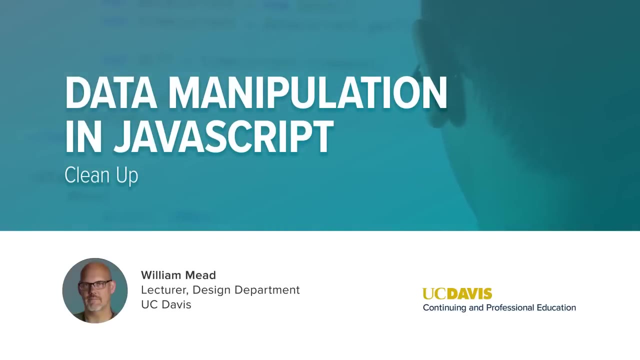 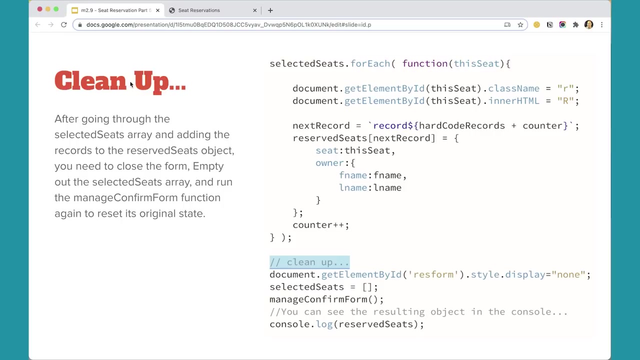 So it is actually working and it's adding those seats into that object up at the top of the page when I submit the form. So that's great. Next, we're going to just do a little bit of cleanup that we need to do in order to get everything back to the same state it was before. we reserve some seats, in case we want to reserve some more seats. 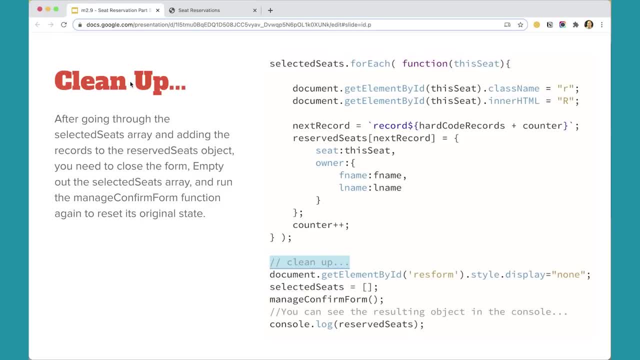 So it's always a good idea. It's always a good idea to return things to the same state they were in originally. So what I need to do first is set that confirm form back to style display none, because after I reserve my seats you can see it stayed open. 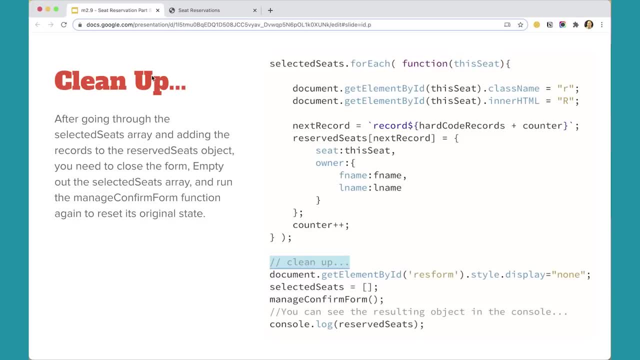 So that's kind of silly. We don't want it to stay open, So we want to set that back to display none. We need to empty out the selected seats array just by setting it back to an empty array And that'll just remove anything that's in it. 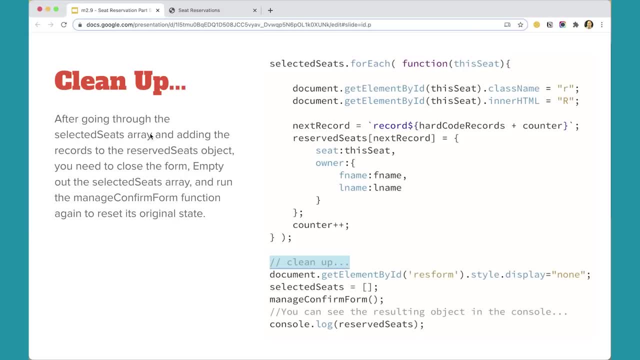 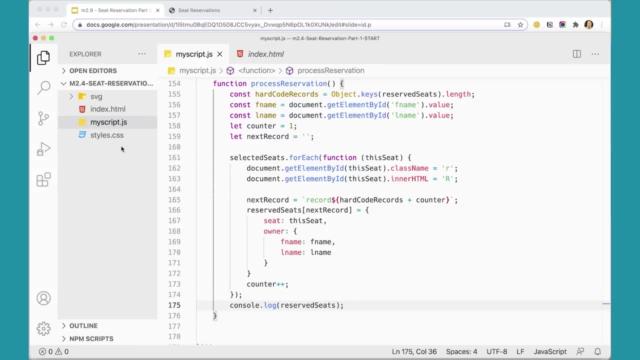 And then it's probably a good idea. You know, we can run the manage confirm form function again, just in case somebody just clicks the button to reserve seats after having not selected any new seats, so we can run that function again. So let's go ahead and add this into our process: reservation function here. 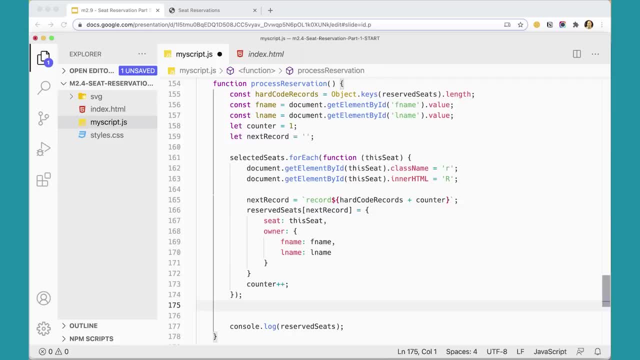 I'm going to put it just before this console log. I'm going to leave that in because I think it is helpful to see that sort of coming up there. But I'm just going to set document, Get element by ID, And the ID that I want is this entire res form here: 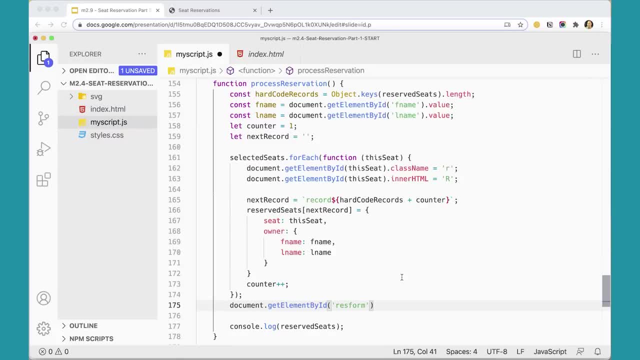 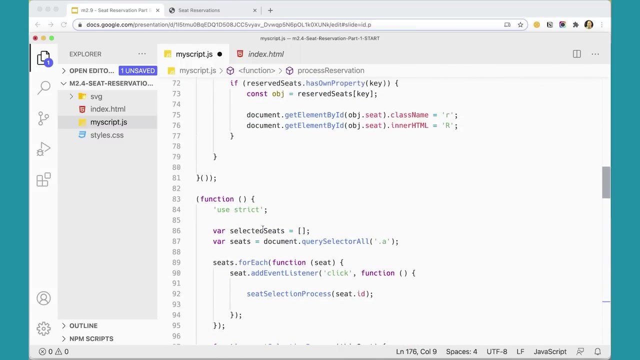 I want to set that back to styledisplay equals none, So that it closes it, It gets it out of the way. And then we're also going to empty out this variable up here, the selected seats variable. I'm going to empty that out. 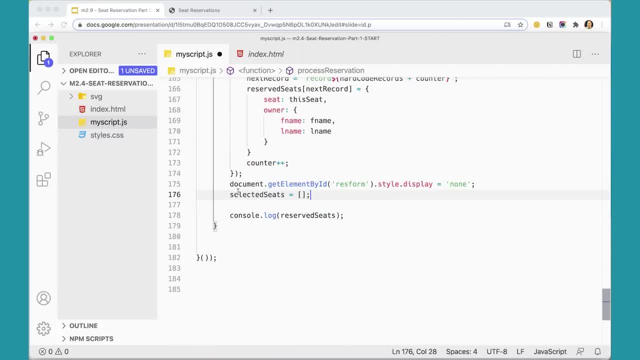 So it's back to none, So I'm going to just set that back. So it's empty. Selected seats is empty, So that's great. And then we're going to run the manage confirm form function one more time, just in case somebody tries to go and reserve some more seats. 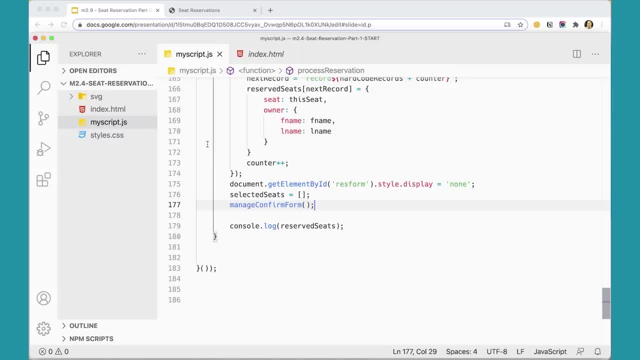 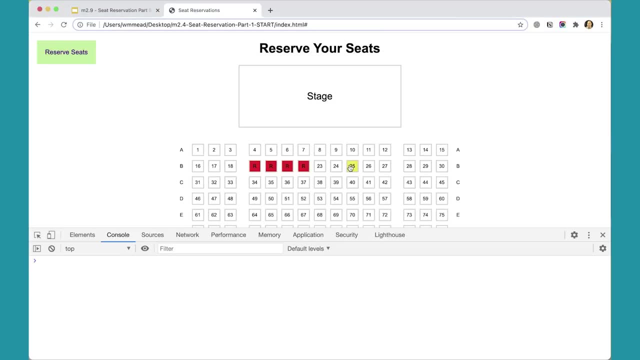 So that kind of cleans everything out and puts it back to the default. Let's go over and test it really quickly. So again, I'm going to just pick some seats, pick these front row, nice and available, And you can see they're going into my array. 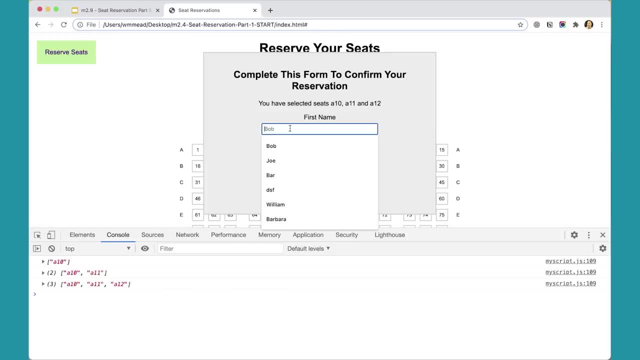 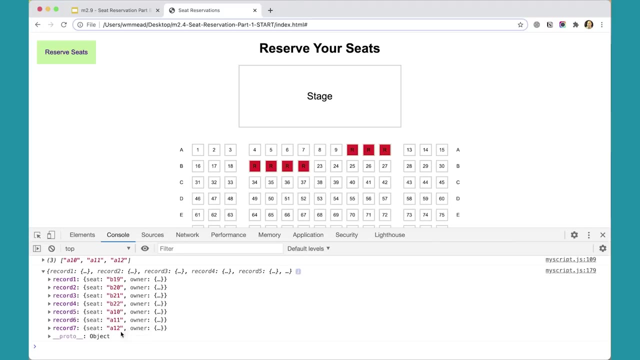 So that's great. I'm going to click reserve seats and I can put in a name- Jose Garcia- and click confirm reservation And you can see I get my records. If I go in here you can see that it reserved these new records and everything's going in and it's working perfectly fine. 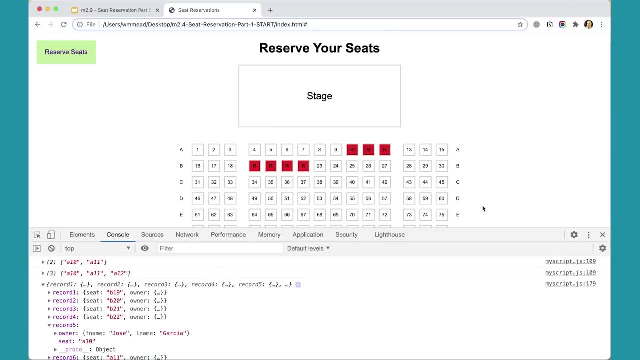 That's cool, Great. Now you'll notice. there's one more minor thing that we need to fix, And that is, after having reserved these seats, I can still come over here and click on these seats again. I close this up. I can click and add these seats again. 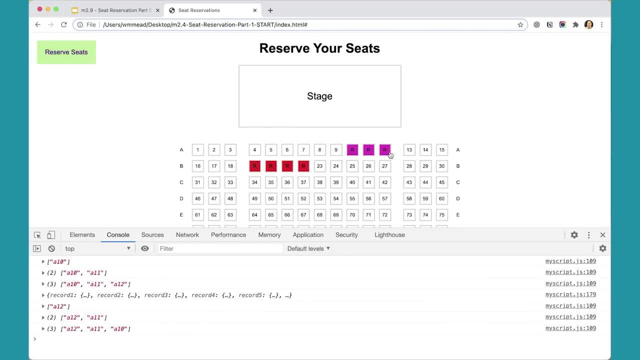 They're supposed to be already reserved, but they're getting added again, And the reason for that is because when the page loaded, these seats were available, So they have the class of day, So they had the event listener attached to them. Now, when we reserved them, we did not remove the event listener from these seats. 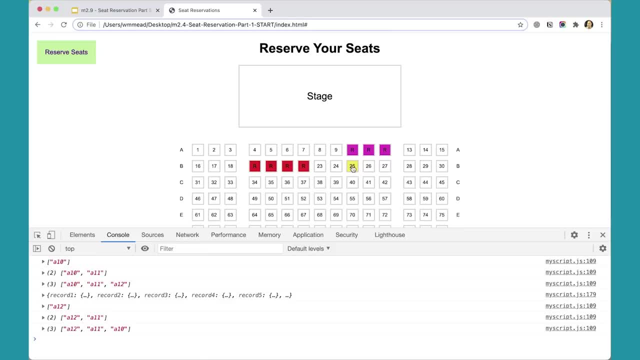 So we need to do one last thing to kind of fix, to fix that potential bug. Okay, So we're going to go ahead and do that, And we're going to go ahead and do that, And we're going to go ahead and do that. 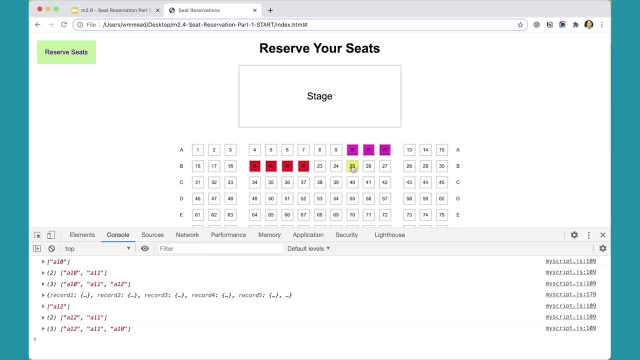 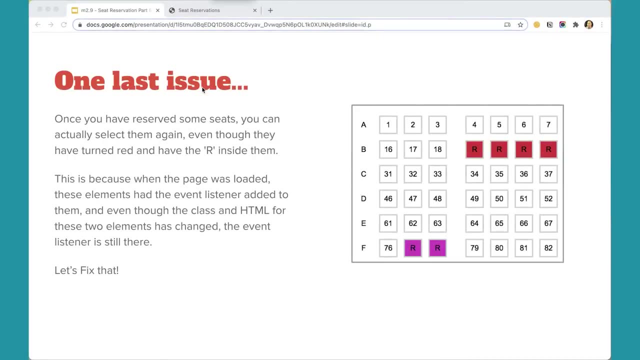 Because we don't want two groups of people to reserve the same set of seats. So how do we fix this last issue? And again, it's because of the way the event listeners were attached when the page was loaded And there's probably a couple ways of doing this. 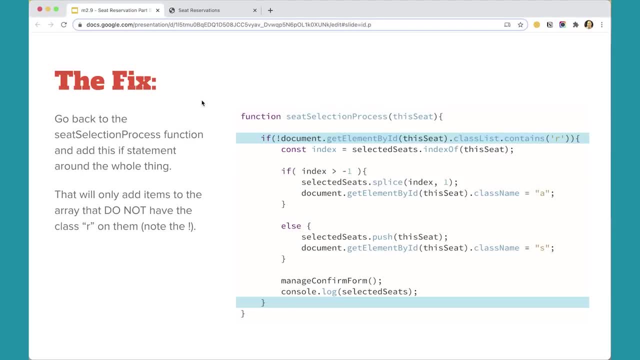 I'll show you my solution for it, Which is to go back to the selection selected seat process function And wrap the entire guts of it inside of an if statement, That's, checking to make sure that the class list contains R If the class, because, remember, we're changing the class from A to S and then to R. 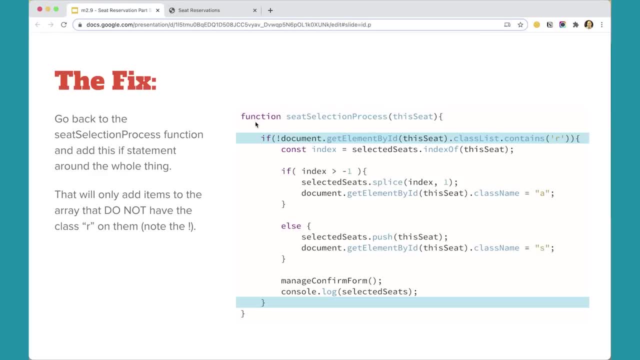 I'm making sure it does not contain R, So you'll notice the exclamation point. So I'm going to make sure it does not contain R. Or you could make sure that it contains R, Or you could make sure that it contains A. 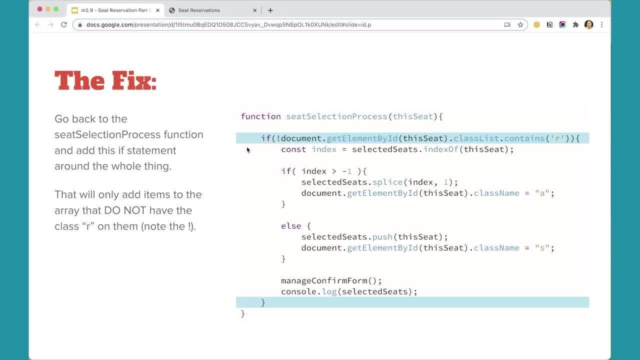 But I'm checking to make sure it does not contain R And I want to go through and do that. I don't want to do the A one because it's possible, Because as we're going through and selecting them, they're going to get changed to S. 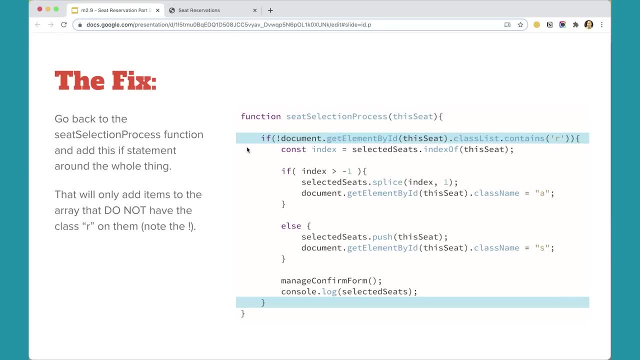 So it would be either. you know, if it contains A or S, it would be fine, But it's kind of more convenient to just check to see if it does not contain the class of R for reserved. So if we just add that, 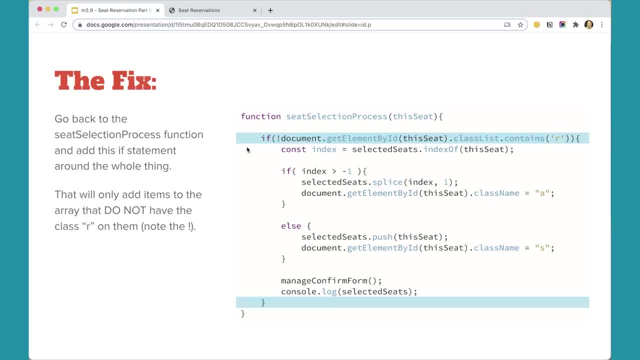 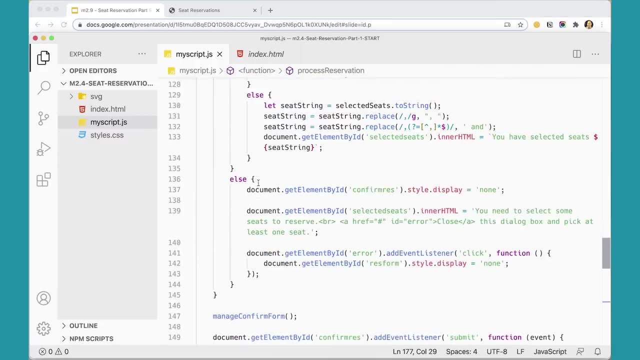 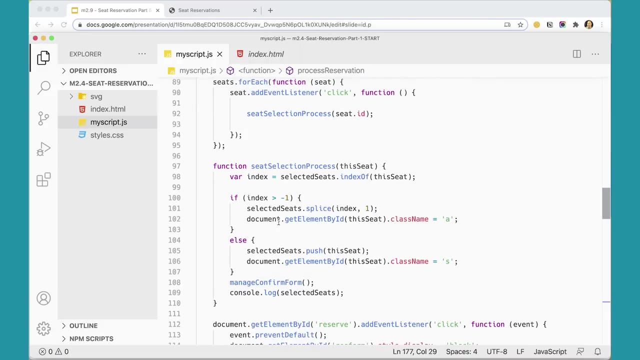 If we just add this if statement in the selection process, it'll all get fixed up. So let's go over and do that. So that's up here in this function Seat selection process, This seat here. So I'm going to put an if statement right here up at the top. 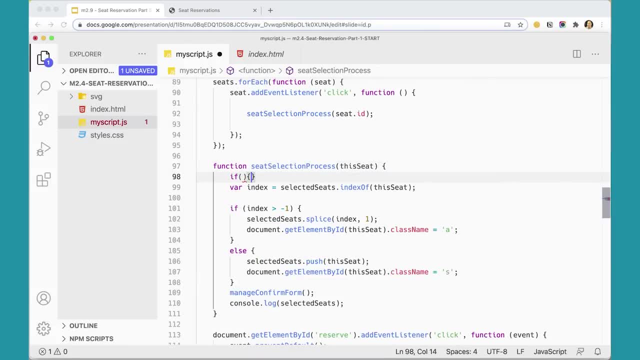 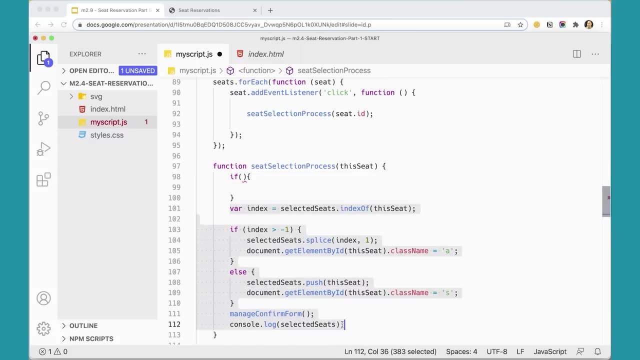 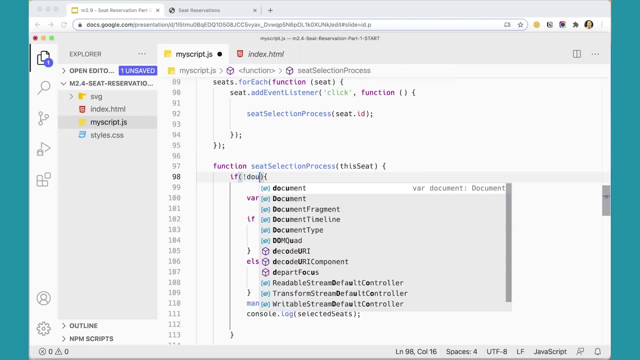 If Like so, And all of this stuff Is going to go inside of that. if statement Like that, And we're checking if not, Remember the logical operator not is an exclamation point. If not, Document Dot- GetElementById. 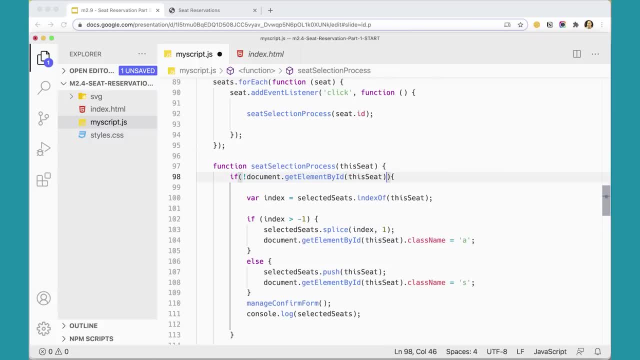 ThisSeat If it does not have classListcontainsR. If that's not true, then we can do this, So let's save that. So Document: GetElementById ThisSeat ClassList. If it does not contain R, then we're good to go ahead and add it to the array. 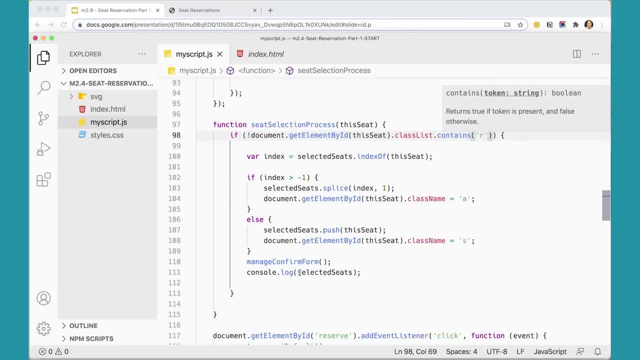 Or take it out of the array as necessary. Okay, So that should be all that we need in order to do to fix this. Let's just get rid of that extra space down there. We get rid of an extra space here. Get rid of an extra space here. 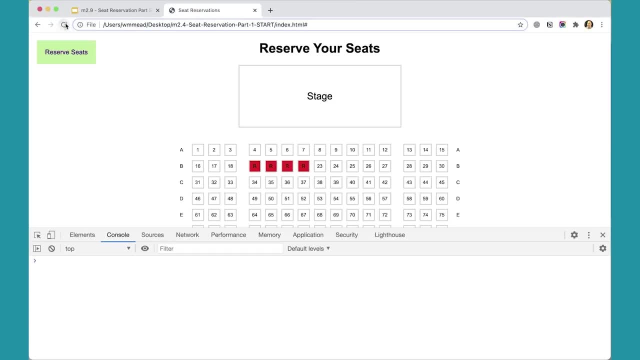 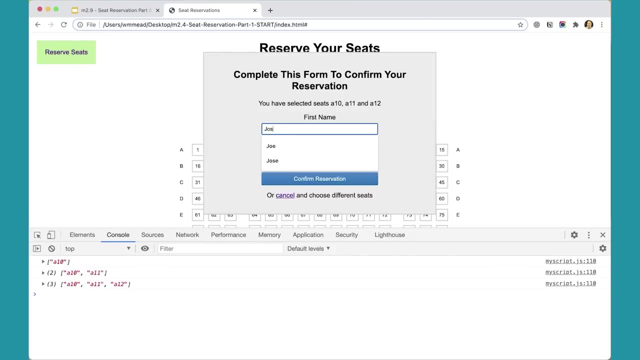 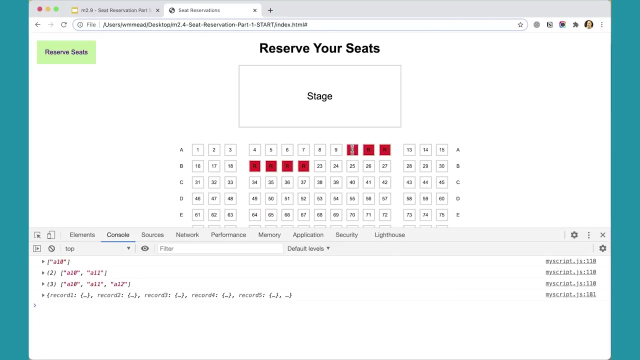 Let's go ahead over here And refresh this And try it again. Reserve seats. Jose Garcia, Confirm my reservation. Those seats are reserved And you'll notice. now I can't click on them. I can click on them, but it doesn't add them to the array. 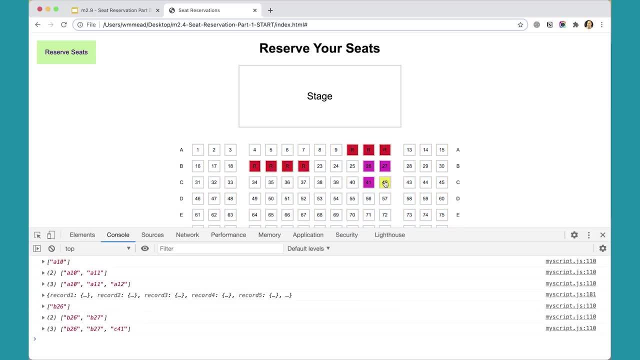 The only thing that adds to the array is I click on other seats, So if I want to go in and reserve some more, I can do that, And everything's getting set back to its original state. Everything's getting set back to its original state. 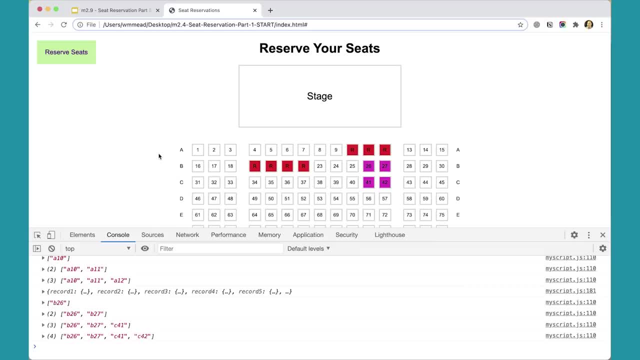 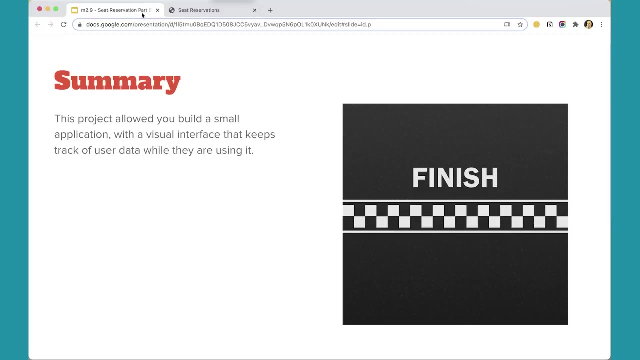 Everything's getting set back to its original state. So there's a lot of pieces to this project. There's a lot to think about, But in the end you end up with a nice little application for reserving seats. And just in summary, here we've created a small web application that does something very simple, but it's got some pieces to it. 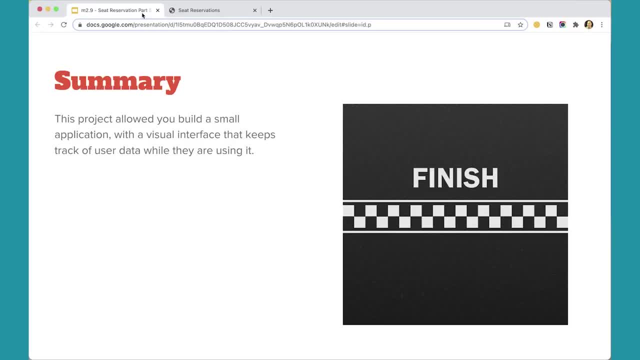 And we were very finicky about the language along the way to make sure that it's clear to the user and that they can't make mistakes. And we were very finicky about the language along the way to make sure that it's clear to the user and that they can't make mistakes. 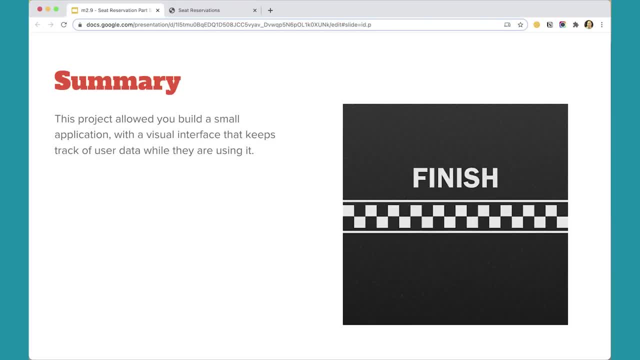 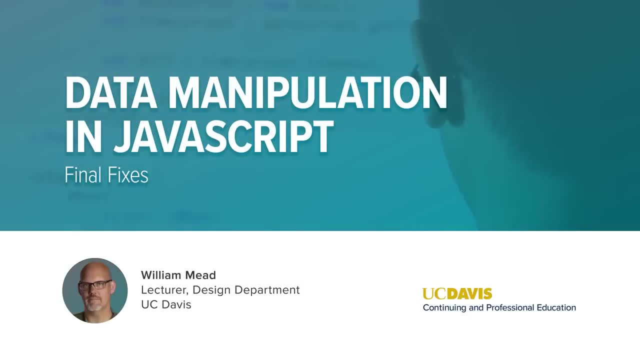 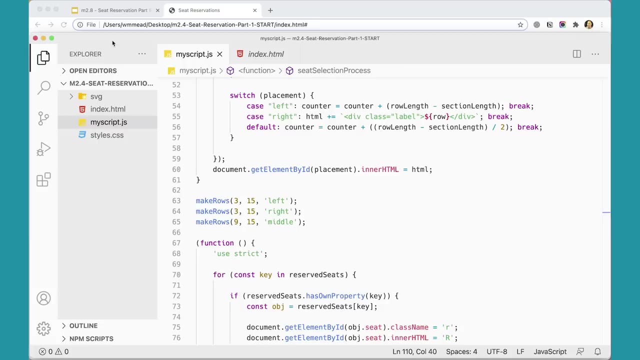 While they're reserving their seats. Great job. Now that the project is finished and it's all working properly, there are just a few minor things that we could do to clean up the code and make it a little bit better in the end. 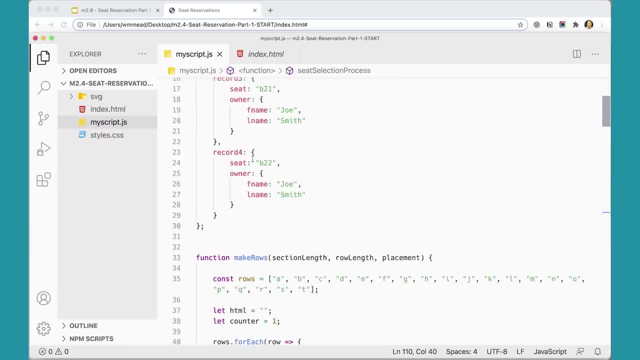 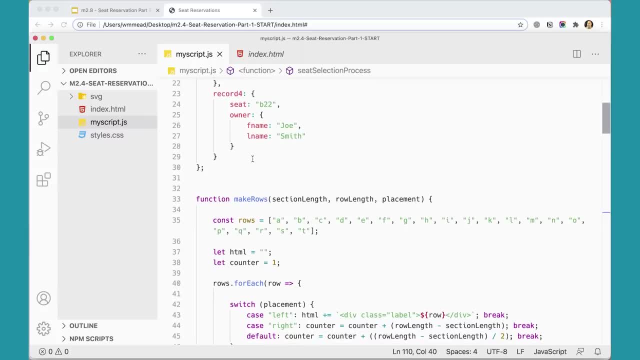 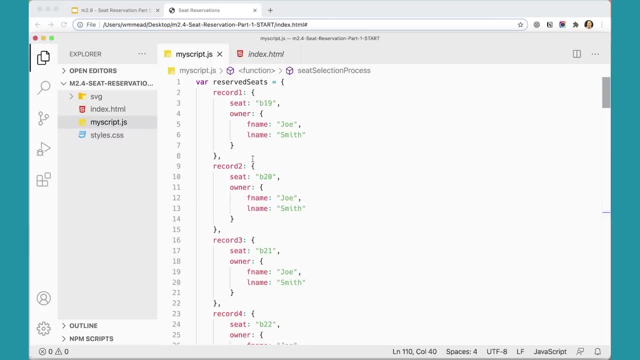 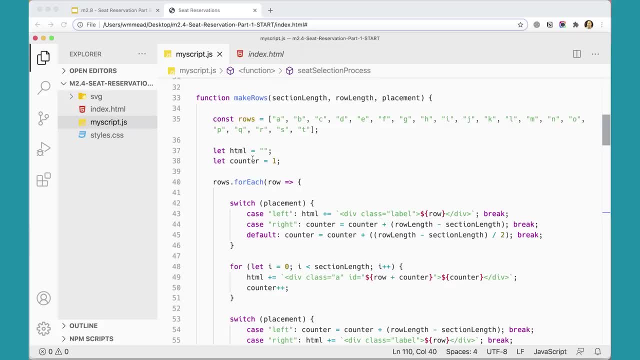 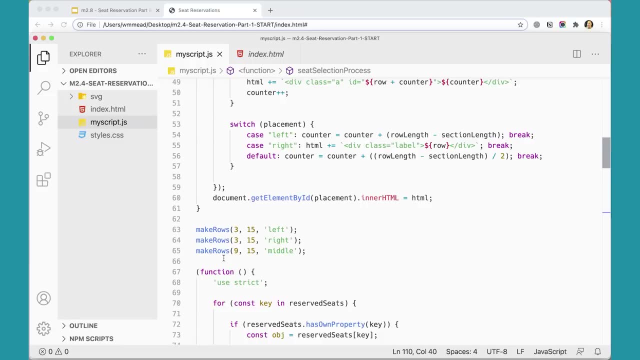 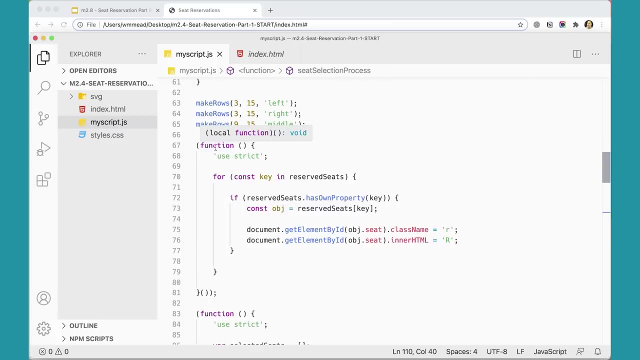 And then we have our function that will generate the interface itself and make the rows. And so we have that function And then we run that function three times to fill in our three different sections of our seating areas. Then we've got a closure, an immediately invoked function expression that closes in this little piece of code here that's going into that object at the top of the page and reserving those seats. 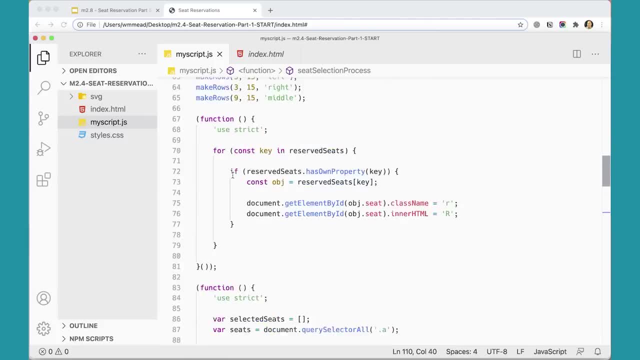 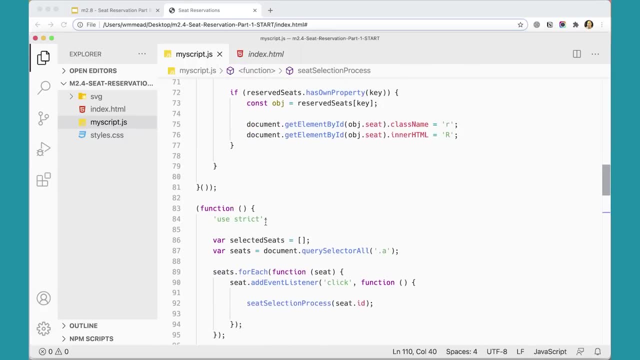 We could, if we wanted to wrap these two functions together, because we've got another immediately invoked function right after that And they really could remove these three If you wanted to and just have this all together. that wouldn't be terrible. 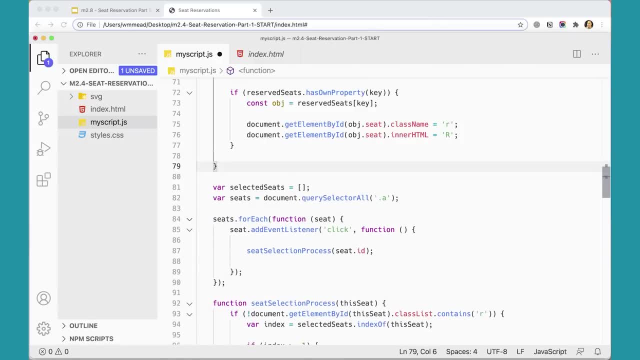 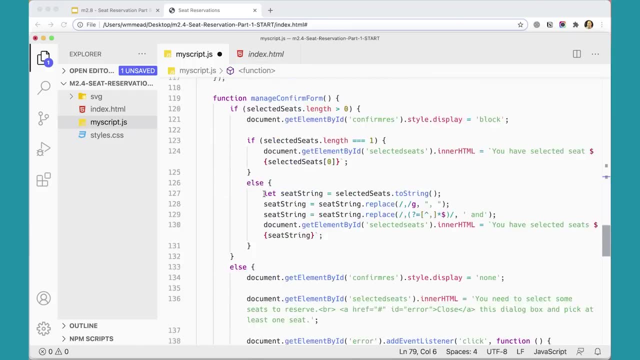 In fact we might do such a thing here. So we're removing the bottom of that one in the beginning of the next one. So this top one here now ends down here at the very bottom of the page, very bottom of the file here. 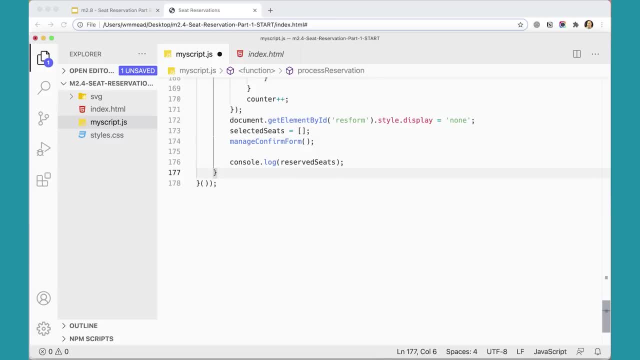 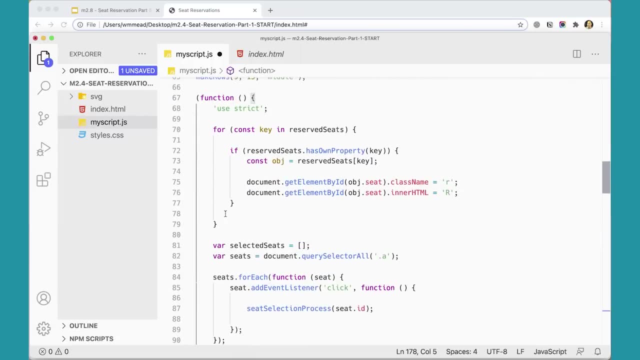 Get rid of some extra spaces there And it's just minor things to kind of clean up and make it, Make your code clear. It's always good to go through and do this kind of thing. You might want to move these variables up to the top. 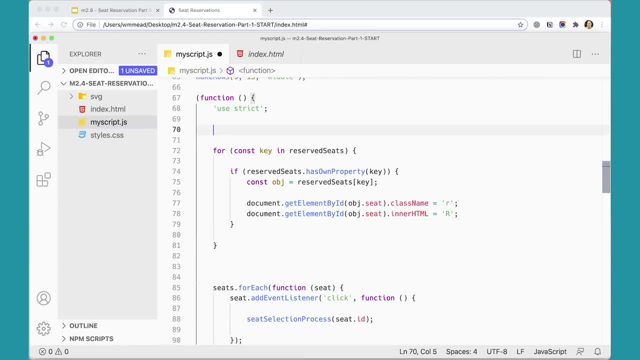 Um, it's. it's always a good idea to put variables right at the top of your script and then to change them from var to either let or const. This one needs to be let because we're resetting this variable down at the bottom. 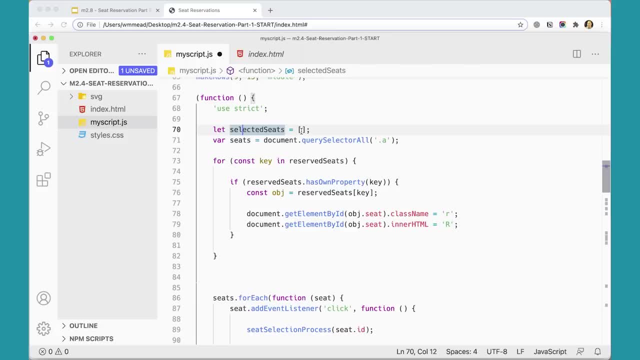 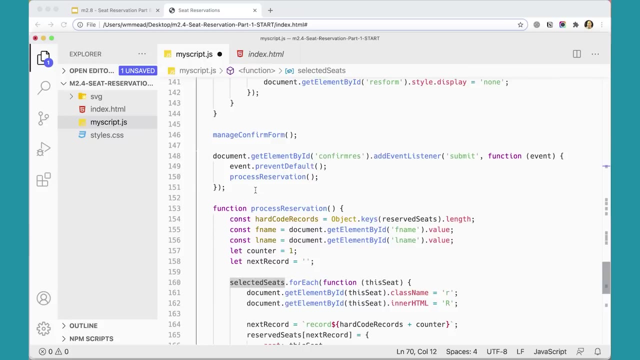 You can. you could leave it const if you were just going to add and remove Um elements into the array. Uh, and you could do that, You could, that could be const. but down at the bottom of the page in the um, in the function for processing the reservation, we're setting this thing back to an empty variable. 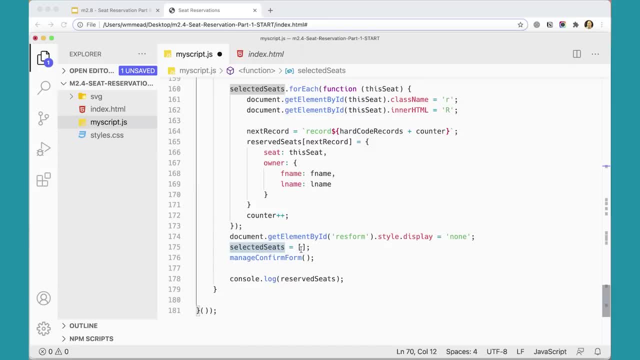 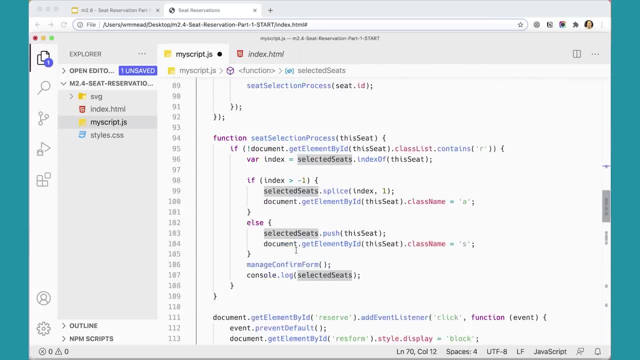 And so if we use let, if we use const up there, then we go to, when we go to do this, it will actually fail. um, because you can't change a variable in that way. Uh, if you assign it. 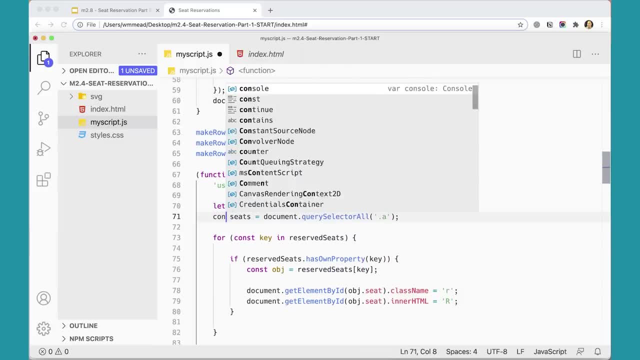 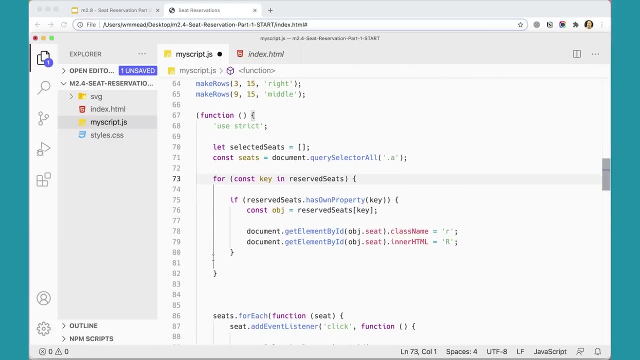 With const. we need let there, but this could be const for sure. And then, you know, I don't know if there are any other places where I used var. I don't think there were, but they, they might come up. 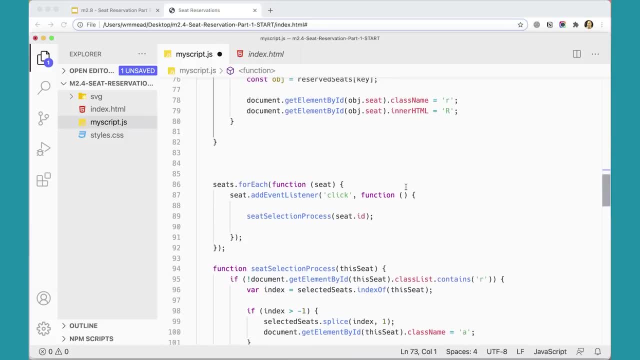 And then the other thing to do is to look for places where you could- and if you didn't do this before, you might want to do it now- where you could replace functions with arrow functions like this. You know, it doesn't really matter. 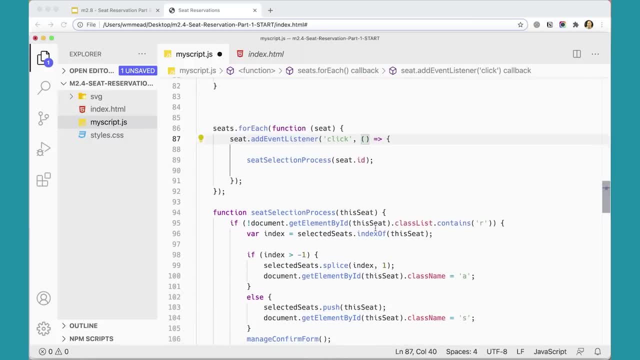 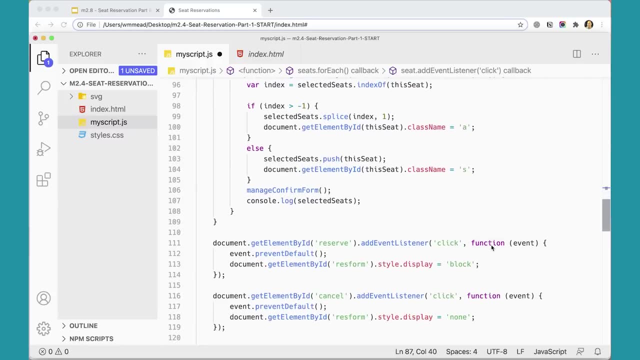 You can leave it with function if you want. but, Um, there may be some places where, if you didn't do it already when we were going through it, where you might actually come in and change these two arrow functions And just kind of clean it up a little bit further and get rid of some of these spaces here. 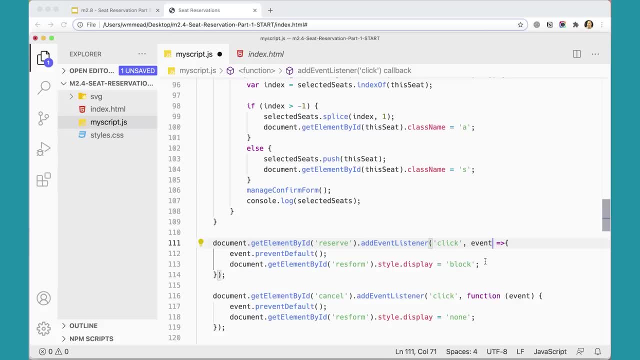 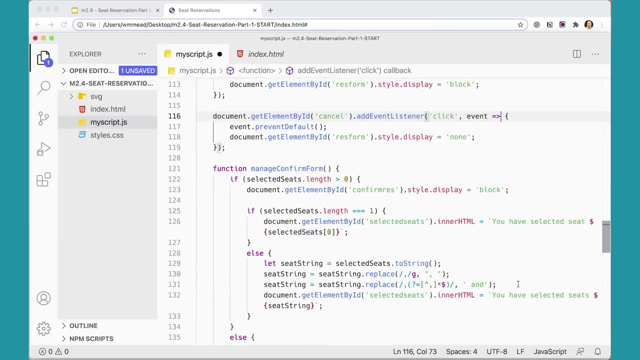 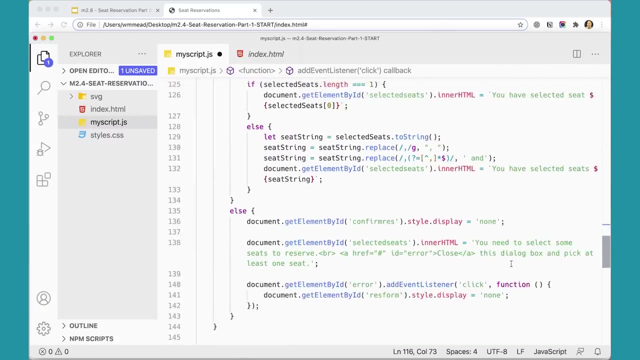 There we go. So we've got a event handler there, Same thing down here. We could actually just copy that And put the same thing here, Um, so that that kind of cleans those up a little bit. go through and look for any other places where I might have used var or where you could do this kind of thing. 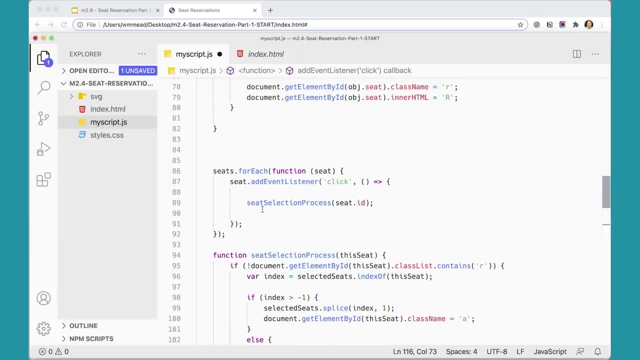 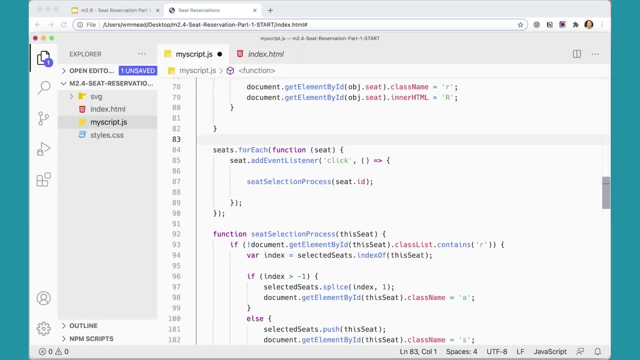 But looking at our code again, so we have um, this foreach is going to go through the seats. Now here. here's another place where we can do this, So we could actually put the arrow function in here and get rid of the word function and then get rid of the seat here. the parentheses here, like: so that cleans that up. 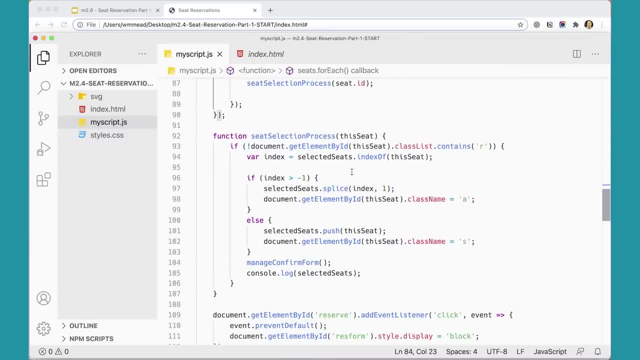 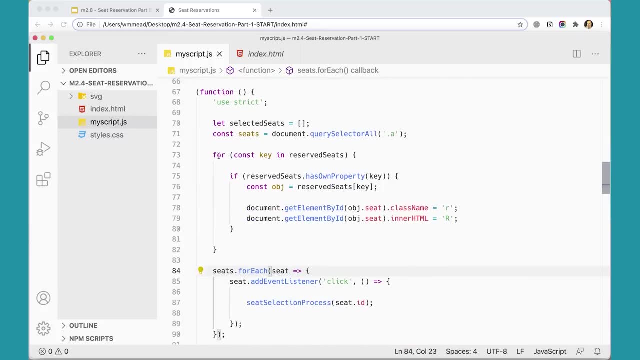 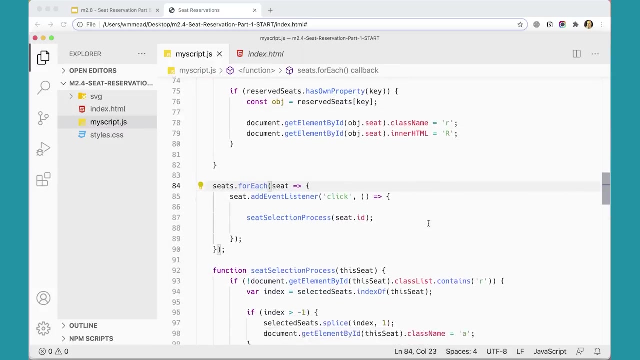 I already have the arrow function there, Um, so you might find some other ones here. Uh, but just going through our code again, we made our rows. We go into our variable here and get that, um, and get the information out of the reserve seats, uh, object up there and and and set those properly on our interface. 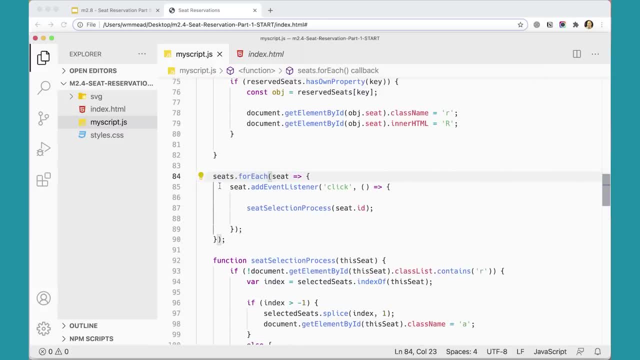 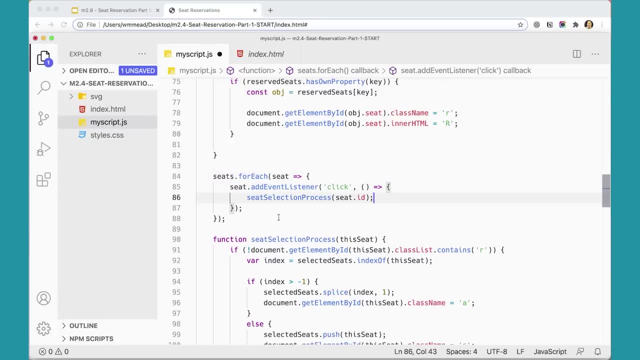 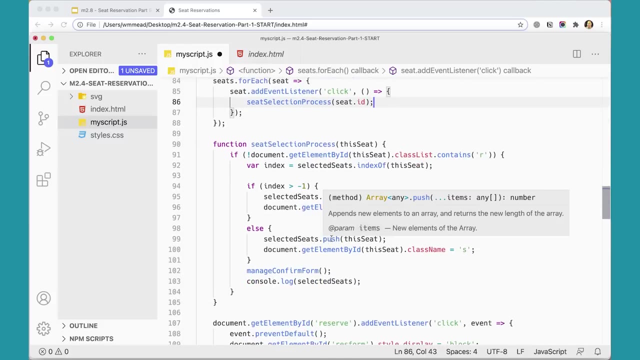 And then we've got a we're. we're sort of looping through all of our seats and adding an event listener. Maybe clean that up a little bit. Um, which is running seat selection process. Our seat selection process allows you, allows us, to add seats or remove seats from the array, updated a little bit to allow us to, to disallow us to further click on seats that have already been reserved. 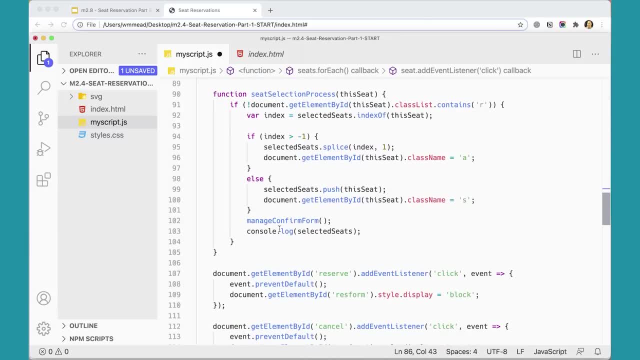 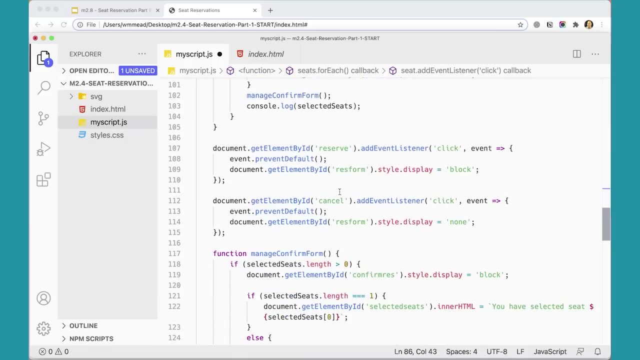 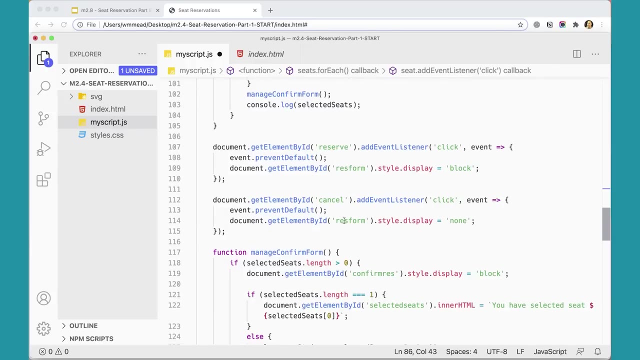 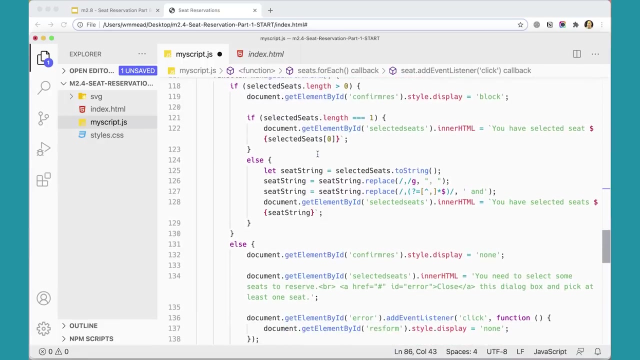 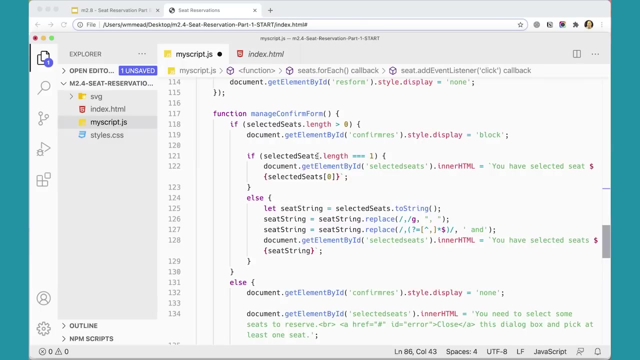 Um, we are running this console log down here as we put seats in the array, So that's worth mentioning. And then we've got some event handlers here for when we click on The uh form element thing, uh, that that'll open and close the form. and we've got our managed conform function, uh, managed confirm form- which will handle whether or not uh which aspects of the form are actually displaying at any given time and how information in that form is displayed. 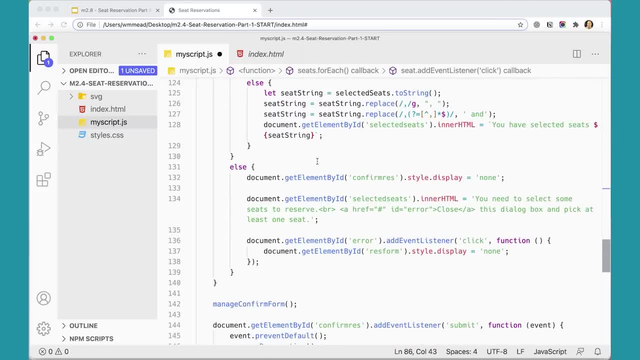 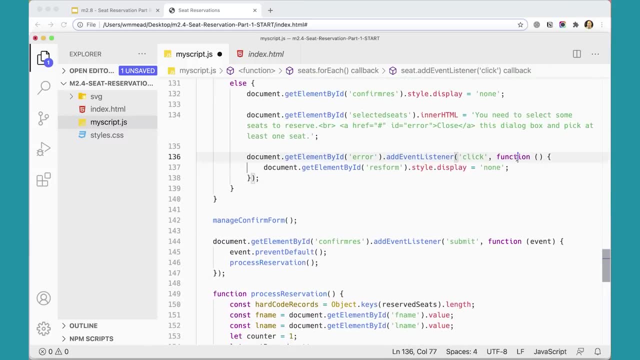 And it's kind of a long function, but it handles a lot of that sort of visual interface stuff. Down here Again, we have another place where we could put in a arrow function. So that's kind of cleaned up a little bit down here. 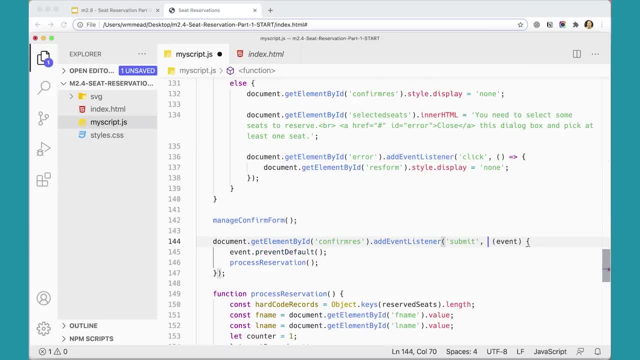 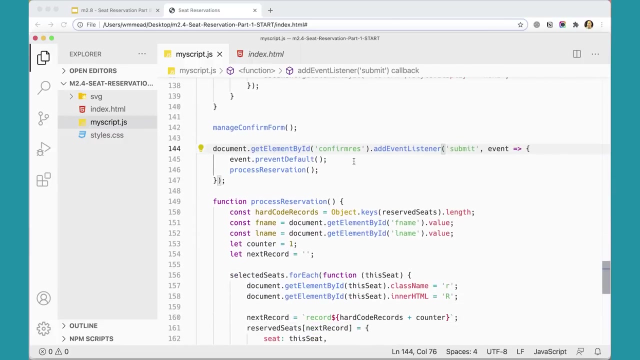 Again, we have another one. It's just good to go in and clean these things up. We've got the event there, Um, so that looks good coming on down here. So now that's the event handler for the confirm reservation process. 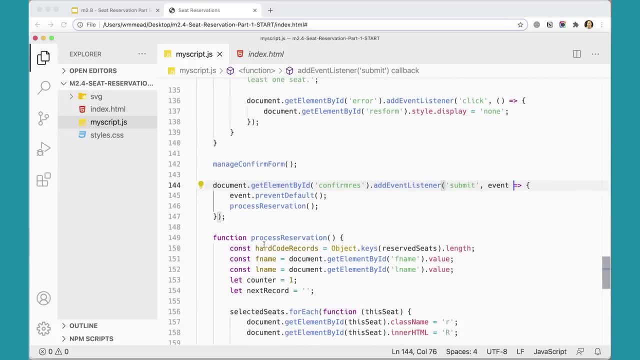 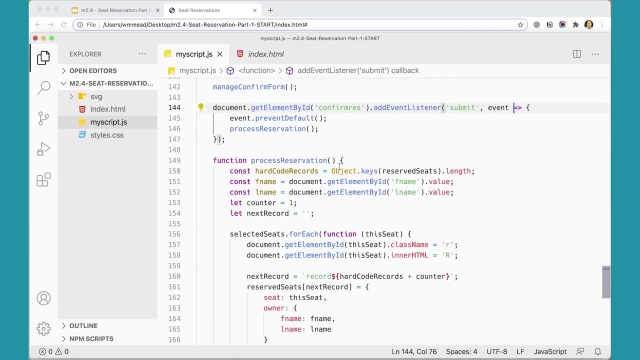 Okay, great, We could group all these event handlers together in one part of the script. That might be a way of cleaning things up a little bit. Um, and then we've got the process- uh, process, reservation function at the very end here, where we're getting those. 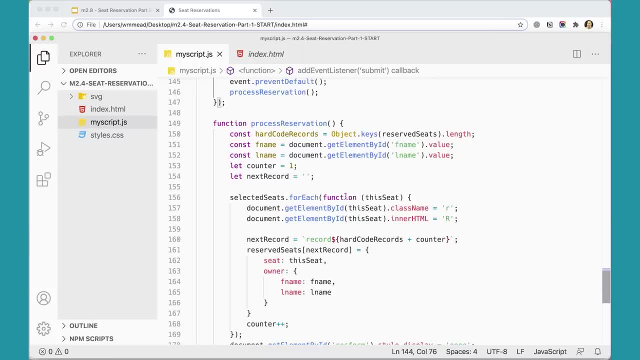 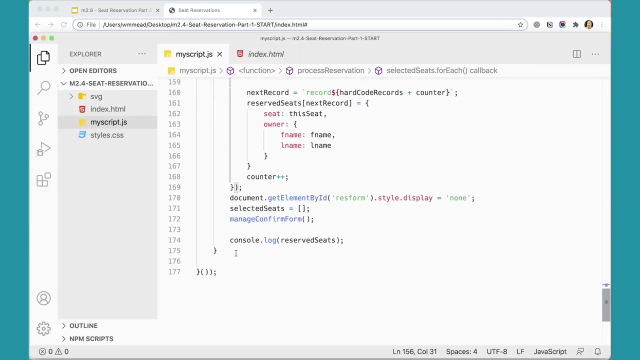 Um records off of the database and then adding new ones. And here's another place where we could change that to a uh arrow function if we wanted to. And again, you might have done some of this as we were going through initially, but it's always a good idea to kind of go through and do it. 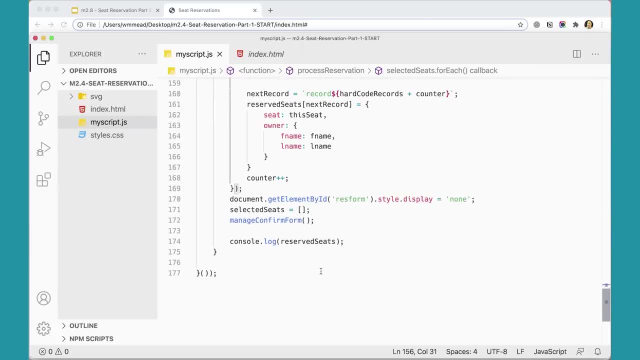 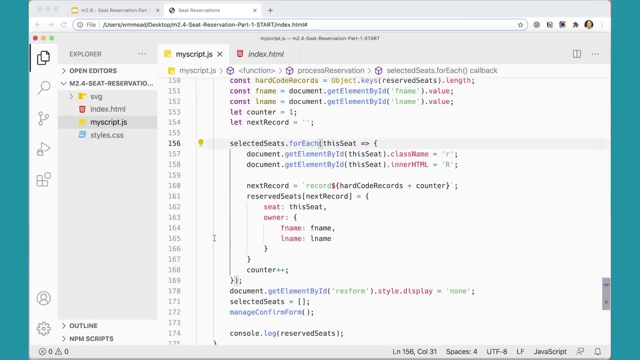 And then, finally, we have the final console log that's showing the reserved seats. So that's our entire script. It's a, it's a big project and, um, it's always good to go through and add it, add in whatever notes you want to add in and make sure everything is nice and clean and organized for later. 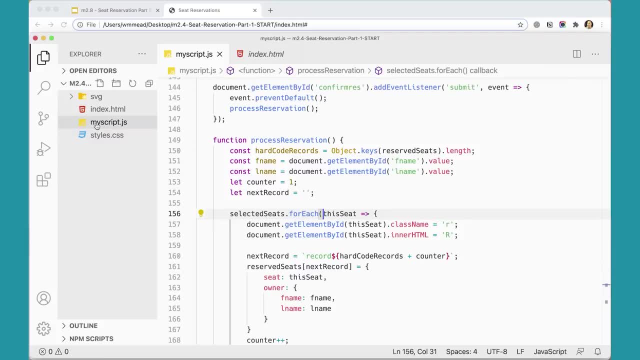 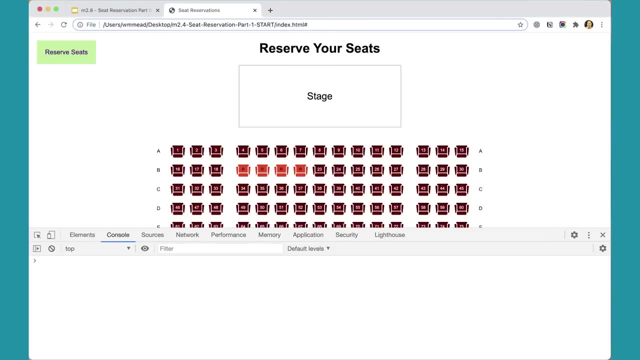 Also, I have another style sheet that you can drop in. If you want to get the actual seats, you can actually drop the style sheet in And that style sheet just has some slightly different styles that are making use of the uh SVG files here of the different chairs. 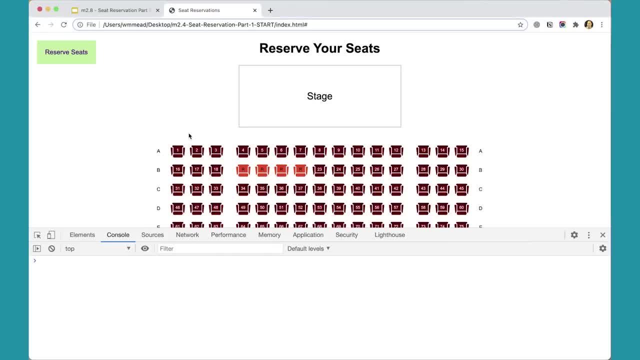 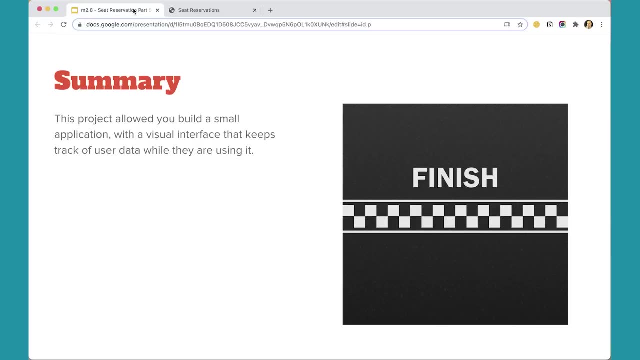 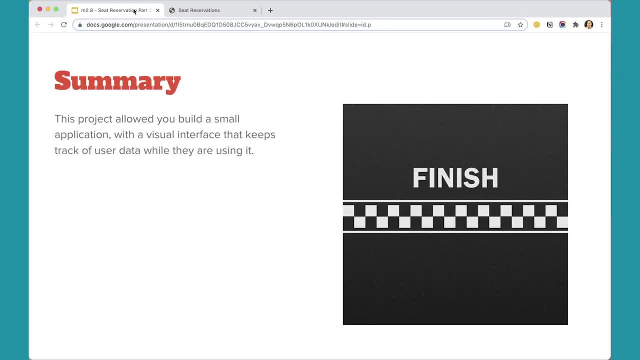 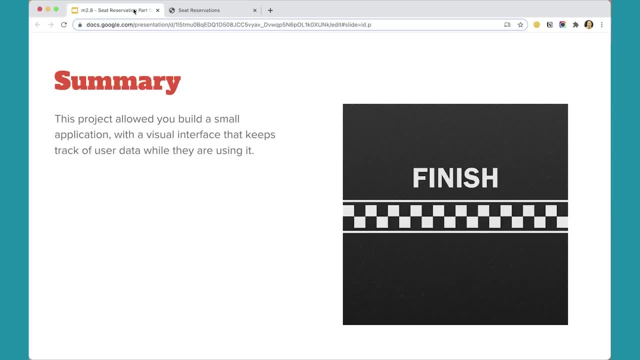 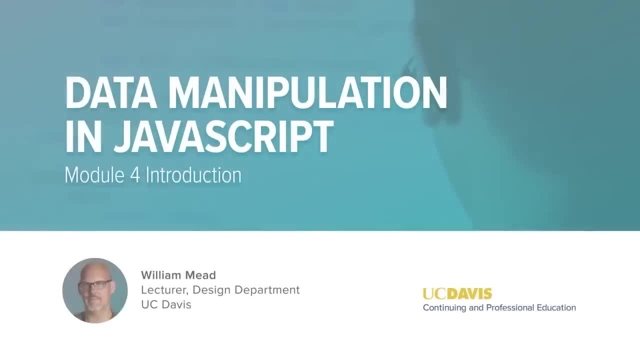 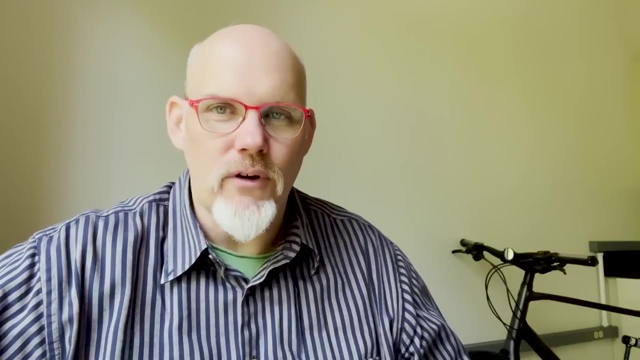 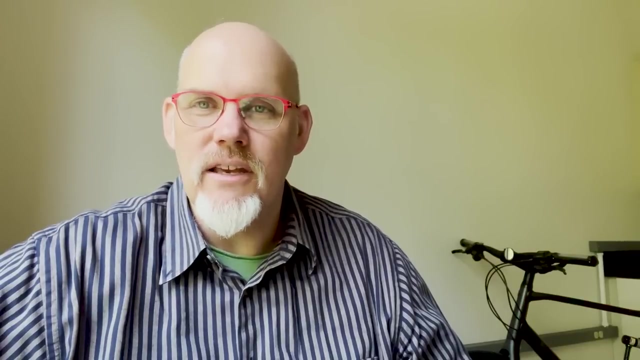 Uh, there are a lot of ways you can take this project and expand on it or do more with it. um, if you wanted to, Hello and welcome to our fourth module for our fourth course on JavaScript. This is our final module and in this module we're going to look at some really great new features that we haven't looked at before. 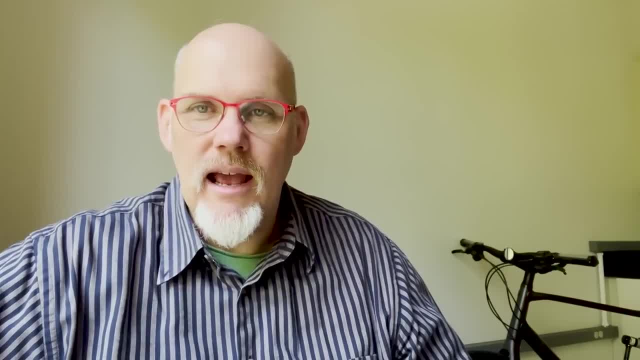 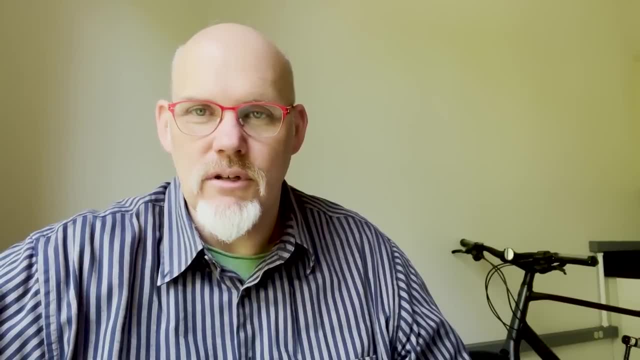 Specifically, we're going to look at asynchronous JavaScript and how that can be used for web projects and bringing in data from external sources and doing all kinds of really cool stuff. I think you're going to get a lot out of it. It's really fun and I look forward to doing this material with you. 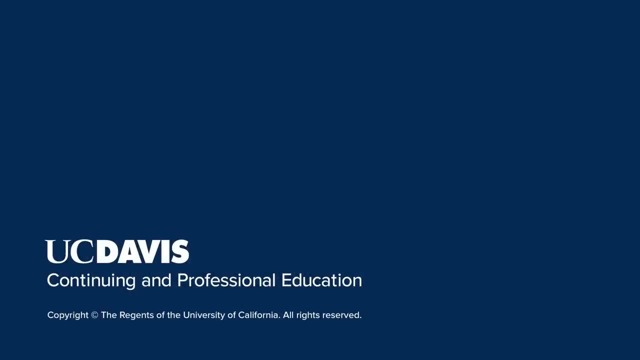 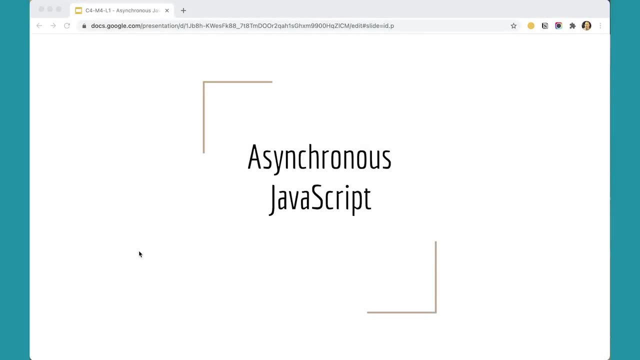 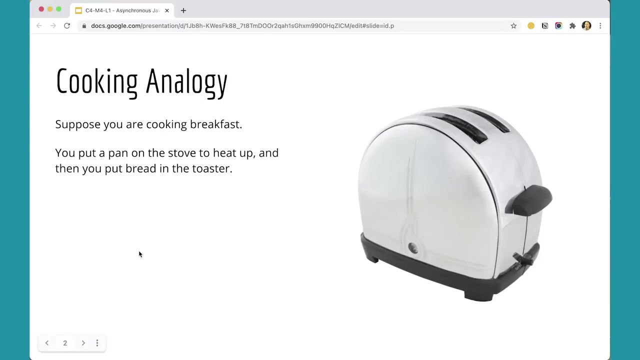 So let's get started. Asynchronous JavaScript. Let's look at a cooking analogy. Suppose you're cooking breakfast. You put the pan on the stove to heat up and then you put bread in the toaster. You don't sit and watch the toaster until the toast is done. 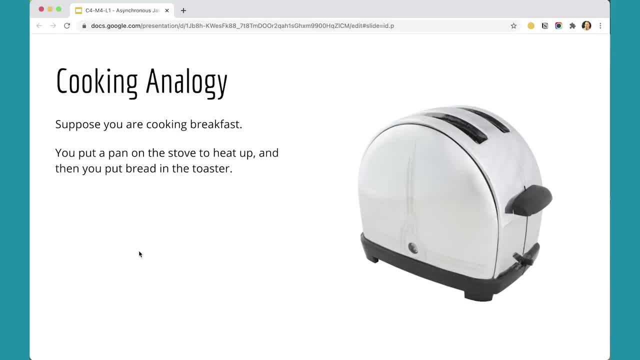 Instead, while the bread is toasting, you put eggs in the frying pan, And then, while the eggs are frying, you pour a glass of orange juice. You have multiple tasks going at once, Each completing in their own time. Back to our cooking analogy. 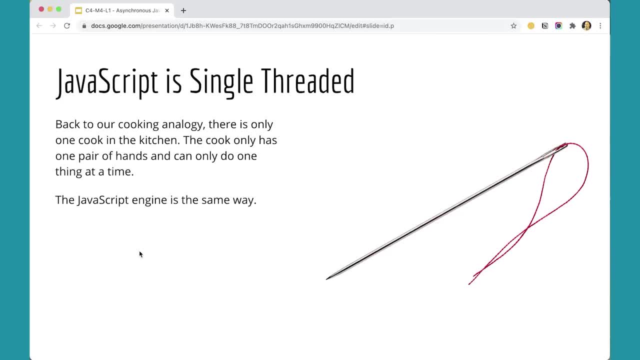 There's only one cook in the kitchen. The cook has one pair of hands and can do only one thing at a time, And JavaScript is single-threaded, meaning that the JavaScript engine is the same way: It can only do one thing at a time. 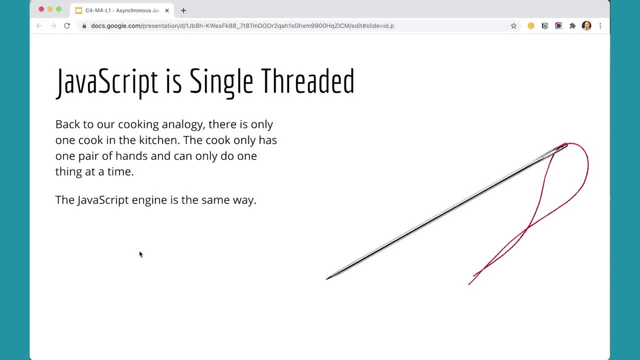 However, that does not mean that it can't start a task, leave it to do its thing and then come back and handle it When it's done. when the bread went into the toaster, the bread went into the toaster and then the toaster bell will ring when the bread is done. 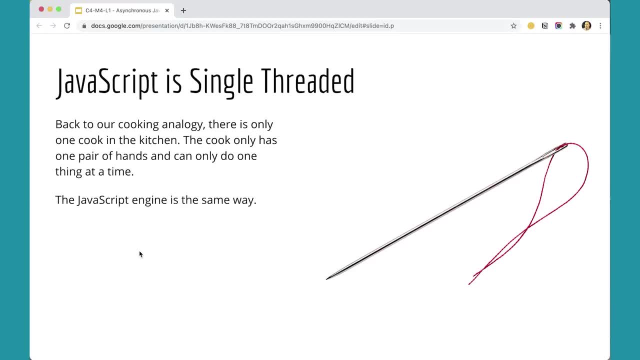 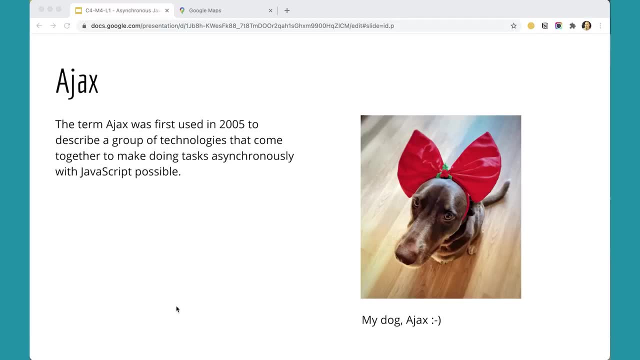 So then, we're ready to. we know that we need to handle that and do the next thing with the toast. Ajax is a term that was coined back in 2005,, and it was developed to describe a group of technologies that come together to create a new technology. 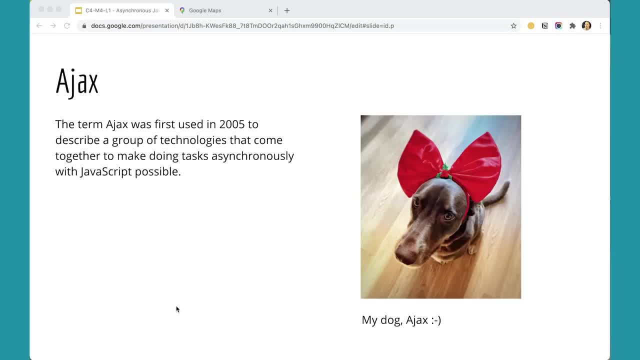 To make doing tasks asynchronously with JavaScript possible, meaning you can have JavaScript go off and do one task and while it's waiting for that to return, you could do another task. It's not. it was not a new technology in itself, nor is Ajax an acronym, but it is short for asynchronous JavaScript and XML. 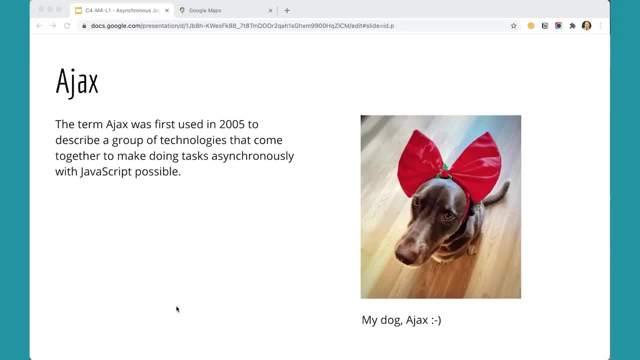 XML is a common language for describing and structuring data, But in fact, Ajax can work with data structure in other ways, Other than other than XML. And, by the way, this is a photo of my dog, whose name is also Ajax. 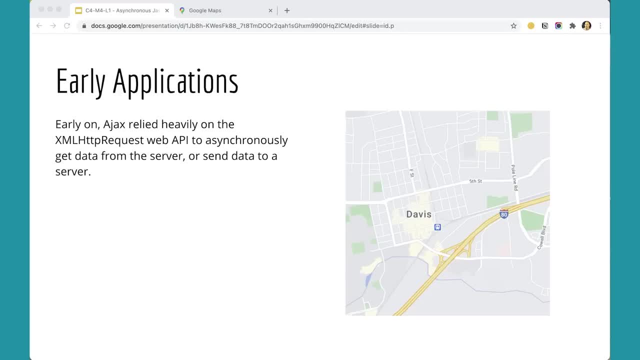 Early on, Ajax relied heavily on the XML HTTP request API to asynchronously get data from a server or send data to a server, meaning it's happening in the background. You can interact with the rest of the page While Ajax is doing its thing. 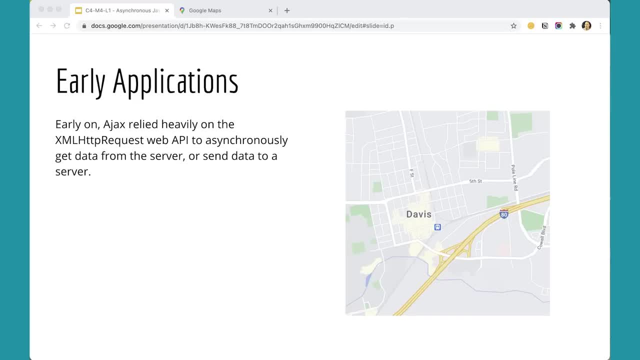 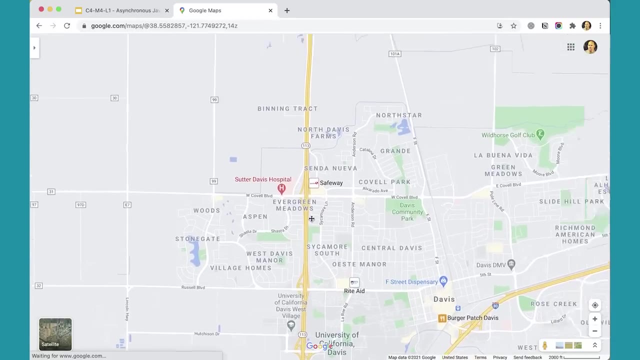 This API was first supported by Internet Explorer five and then it was widely supported by other browsers. Google Maps is an example of asynchronous JavaScript at work. So when you're on Google Maps- and here we are in Davis- you can drag the map around and it will load tiles for new portions of the map, as it needs to. 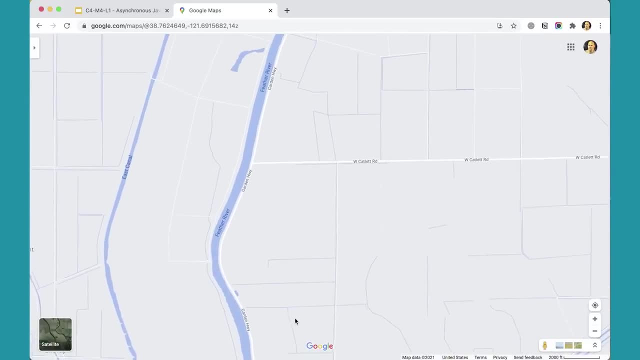 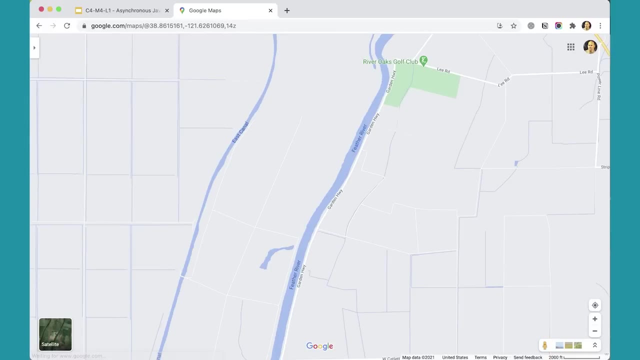 Now my Internet connection here Is fast enough that I can't really see these tiles coming in. but you may have seen it if you're in your car or in a lower data place and you go to drag it. Sometimes you'll see the tiles actually coming into the page as the page loads. 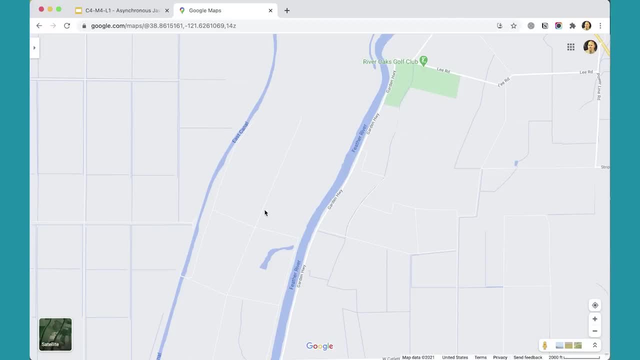 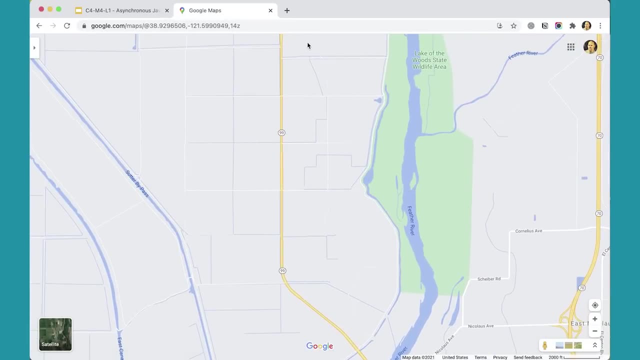 And that's all happening asynchronously. In the old days, with the old versions of web map software, you'd have an arrow on the top. if you wanted to click, if you wanted to go up, you click the arrow And then the entire page would. 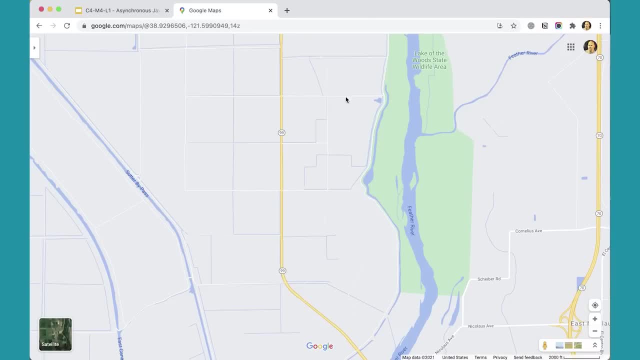 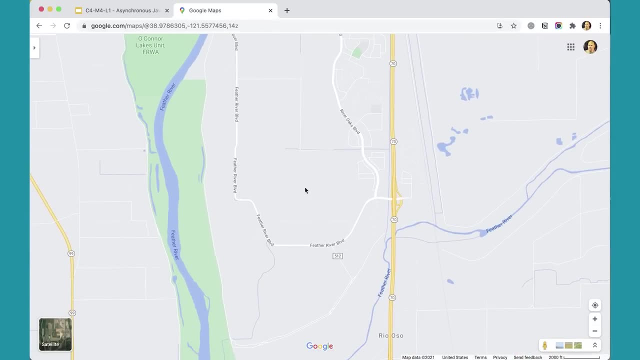 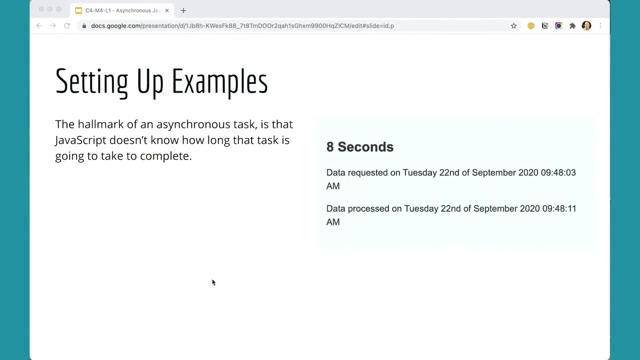 Load with the map up the next section, but that created not as nice a user interface. It was much more difficult to follow exactly what was going on and where you were in relation with that refreshing of the page. Let's set up some examples so we can see how this asynchronous JavaScript works. 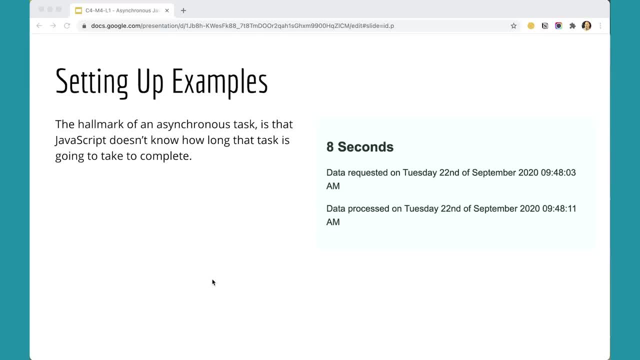 The hallmark of an asynchronous asynchronous task is that JavaScript doesn't know how long that task is going to take To complete. while we, as users, are waiting for that task to complete, we should not be blocked from doing other things on the web page or the web application. 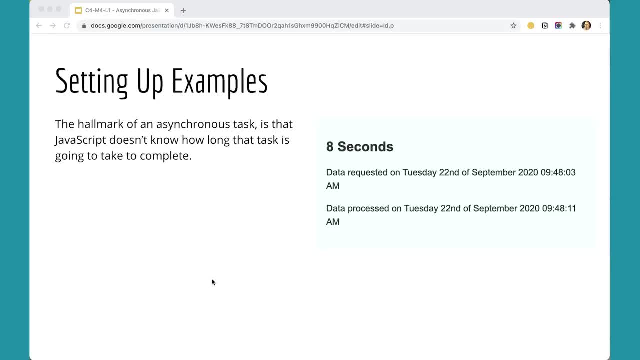 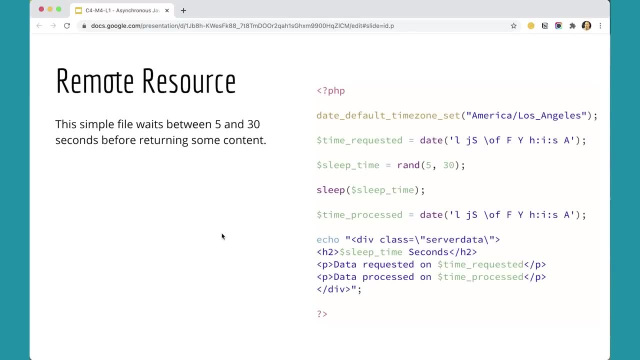 I created a file that randomly takes between five and 30 seconds to process and I put it on my server. It's a simple PHP file and we can see over here. This isn't a PHP class, but I'm setting a time zone. 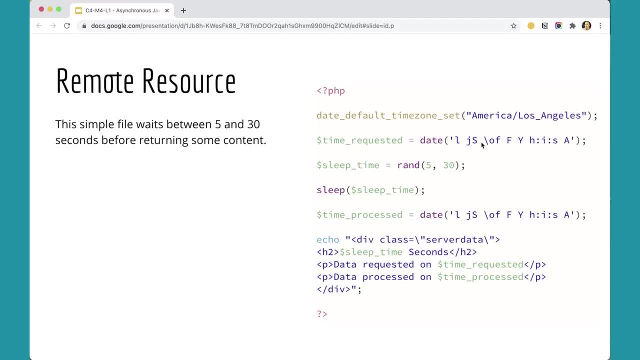 I'm setting a time Requested, which this will generate a date object with a month and day and all that kind of stuff here. Then I'm using a random number generator to generate a number between five and 30, which is going to represent seconds. 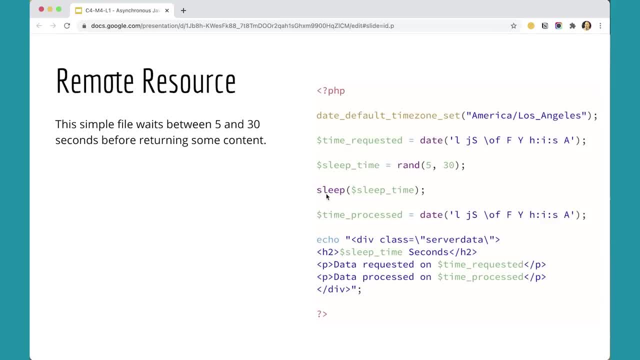 And I put that in sleep time And then PHP has a function called sleep which will just make it wait for a period of time. So it's going to wait between five and 30 seconds. Could have put the ran 530 in here. 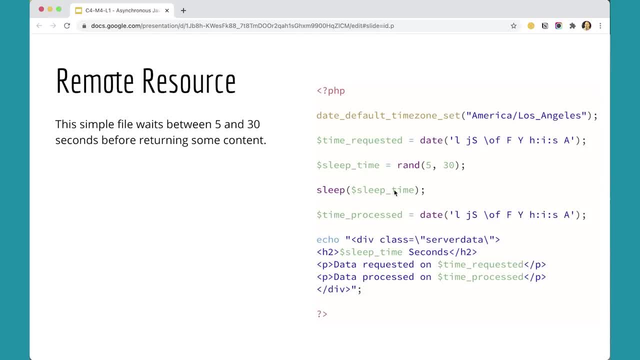 But Yeah, Yeah, Yeah, I wanted to make it clear that this is sleeping, however amount of time that is. And then I set another variable with the time that it was processed, And then I print these out: div class server data. 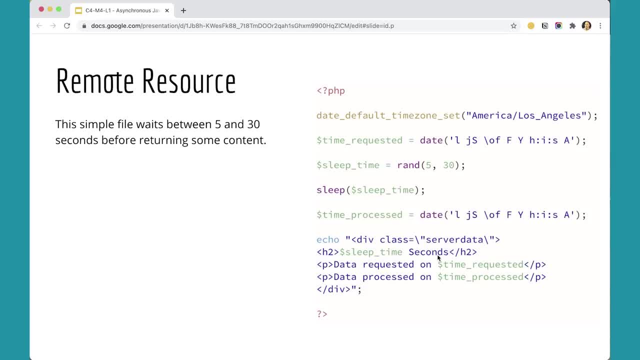 I'm doing an H2 sleep time and, uh, the number of seconds that it was set to sleep inside the H2. And then I'm just printing out the time that was requested and then the time it was actually processed And you can go to this web page on your um. 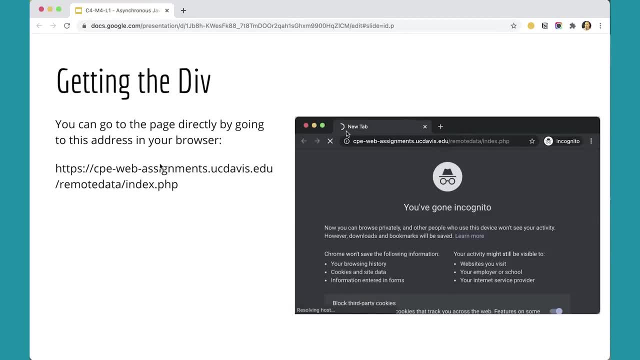 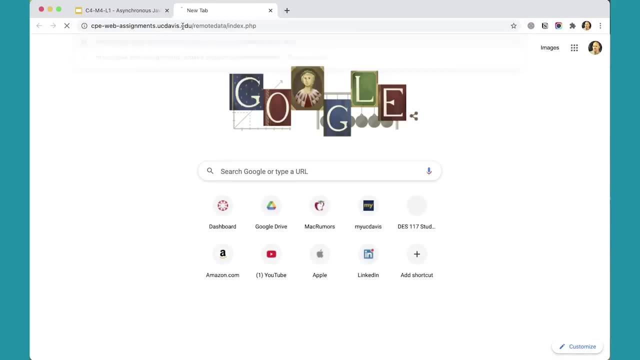 On your server. here we can actually go to the CPE, CPE dash web assignments- ucdavisedu slash- remote data slash index PHP. So if we do that, then you'll see what will happen is if I put in this URL, this thing is going to spin for the number of seconds that that thing has been set to sleep. 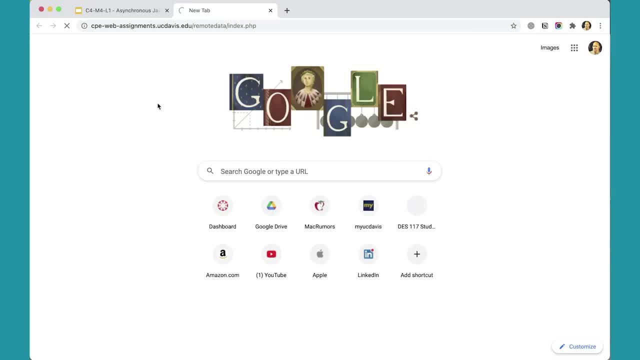 And it could be five seconds, It could be 10 seconds, It could be up to 30 seconds long- that we're waiting for this page to load because PHP is is set to go And it actually waited 18 seconds there. 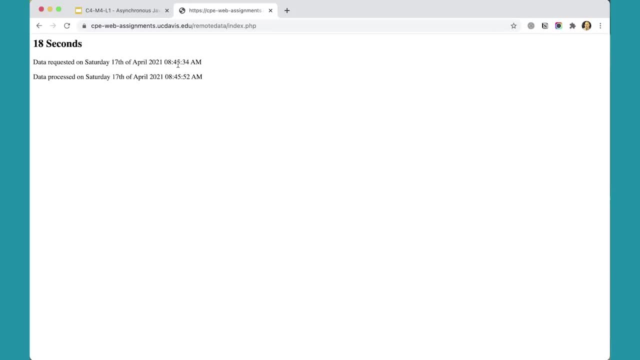 And I can see the date requested: 8: 45 AM with 34 seconds, And then 18 seconds later you can see 45 at 52 seconds. It was actually processed. Now, if we work locally with JavaScript, we won't have to wait. 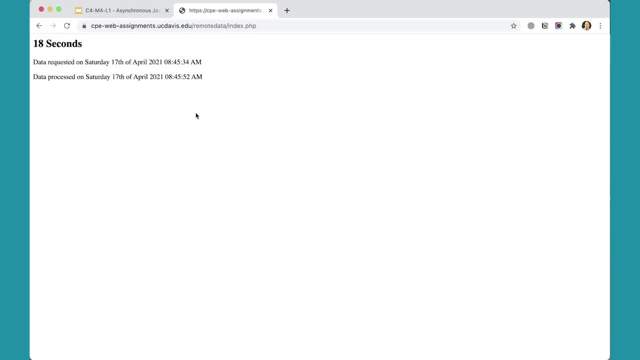 For this to load. We can have the JavaScript page, We can have an HTML page using some JavaScript- uh, waiting for that to happen- and then return the data to us when it actually does. So let's try and play around with that in the next video. 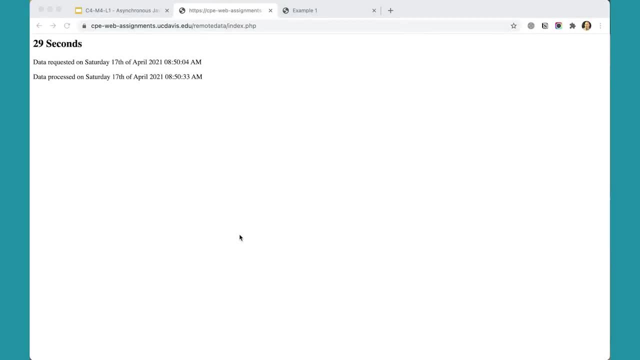 In the last video we looked at a file that Takes between five and 30 seconds To process, And each time you refresh the page it could take a different amount of time. This time it took 29 seconds. One last thing I want to quickly show you before we move on from this file is that if you view the page source is that it's not an entire HTML file. 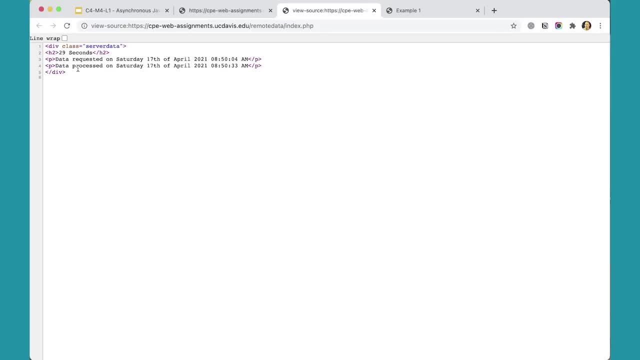 It's just a div, So we could take this and like include this data in another webpage if we wanted to, because it's not an entire webpage, it's just part of a webpage. So that's kind of an important thing to understand about the way this file is constructed. 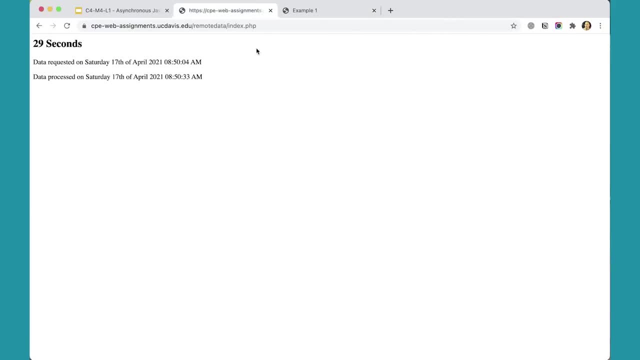 The other thing I want to make really clear is that if you load this page up directly, you have to sit and wait for the browser to finish, uh, waiting out this timer, however long the timer is- And uh, 20 seconds is an interminable length when you're sitting and waiting and just looking at a blank page. 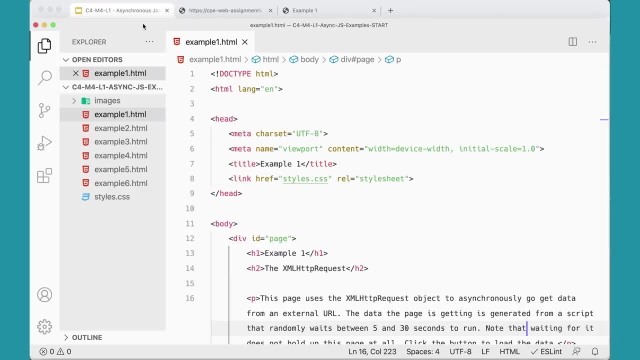 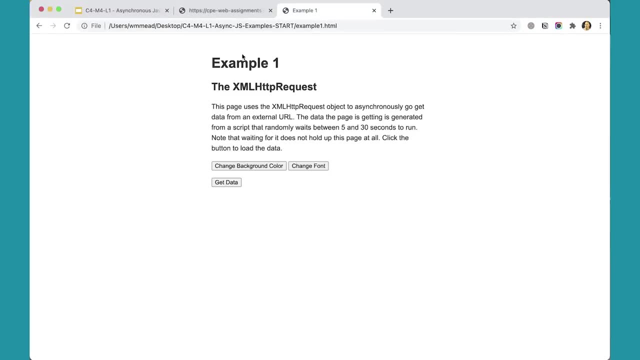 If you go to the start files for this last time And open them up in your code editor. Let's take a look at example one, and over here I have example one displaying here. It's not going to work yet because we need to add some JavaScript to this first, but this is example one, and we're going to just look at the XML HTTP request JavaScript object that will allow us to get this data asynchronously using old fashioned uh JavaScript to do that. 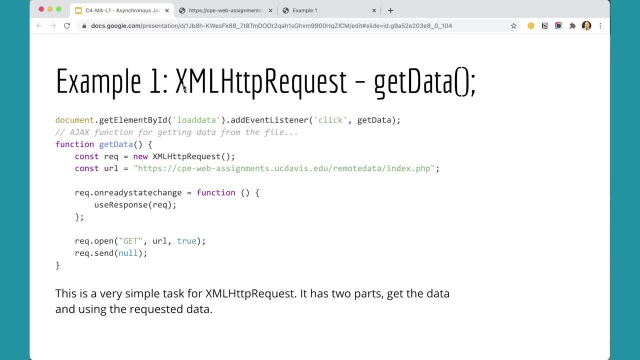 And um. so yeah, we're going to use the XML HTTP request to get data, but this is a very simple task. It has two parts: get the data and use the requested data. The open method uses the get HTTP method and the URL to get the data from the URL. 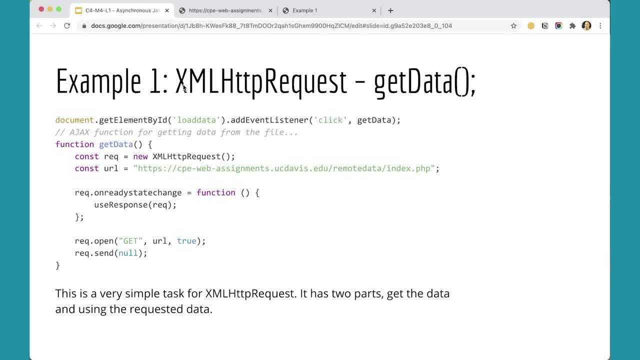 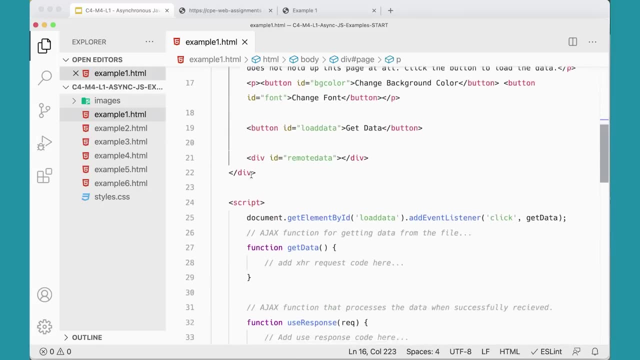 The true flag indicates that it should do so asynchronously. So that's what's going on down here. We're going to have to put this into our code over here. So if you come down the page here, we need to add that in here. 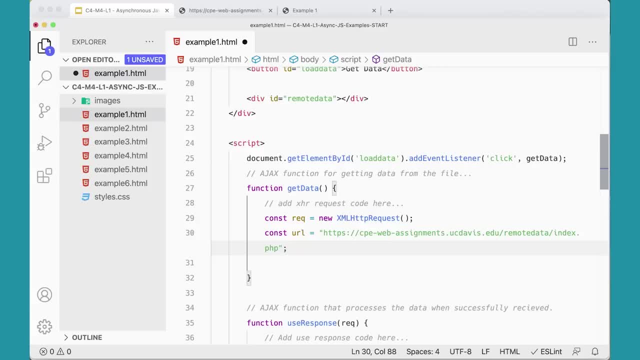 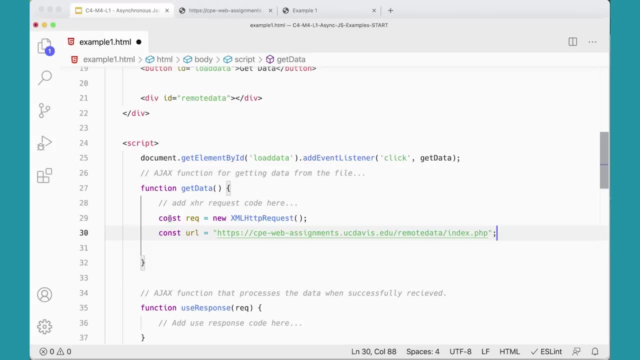 I'm going to start by adding two variables here. I'm going to close my Explorer So that doesn't wrap around, and I'm going to. I can see, here I've got, I've got a variable for REQ, which is going to be a new H, X, M L HTTP request object. 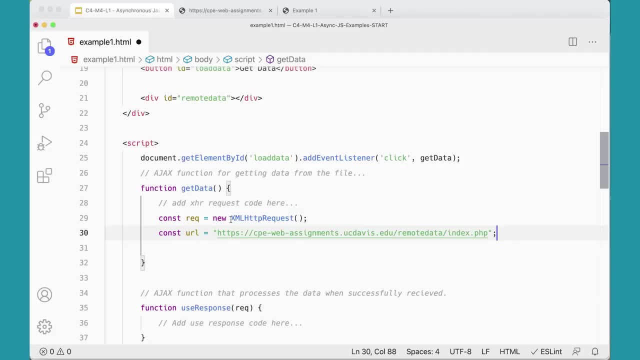 It's a mouthful, but that's what that is. It's a new XML HTTP request object, And then I've got a variable for the URL, And this URL is the one that is the PHP file that we're looking at on the server, the piece of a webpage. 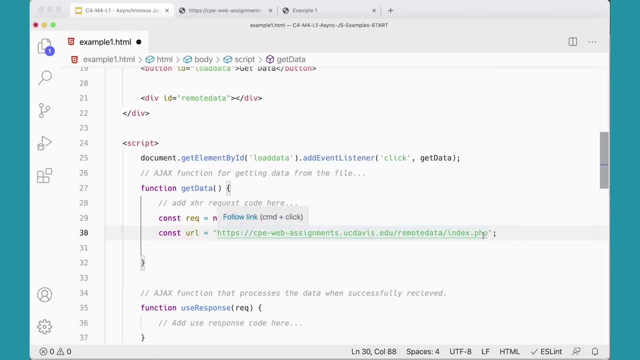 It's just that div that takes a while to load. So that's where we're going to go Request And then we're going to have to add some data from Then the, the XML HTTP request object has a method called on ready state change, so that this is going to happen when the data is ready. 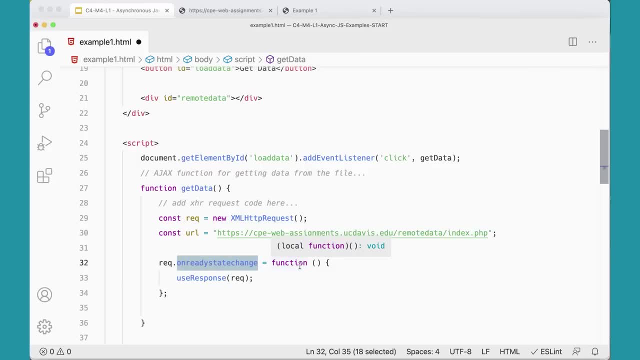 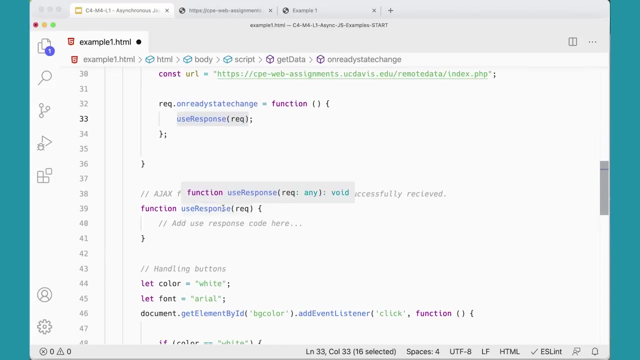 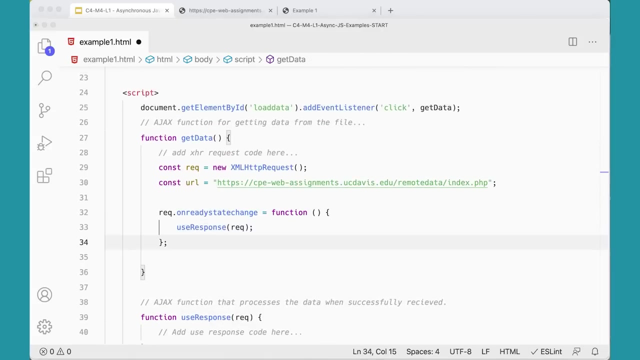 Once it's got some data, it's going to run this function and it's going to run a function called use response And we're going to pass in that Request object when the when the data is ready, uh, we'll be adding this function down here. here's the user response function, and we'll fill that one out in a minute so we can actually see what that does. but this is the asynchronous bit, because this is the part that's waiting for something to change, waiting for us to get the data. 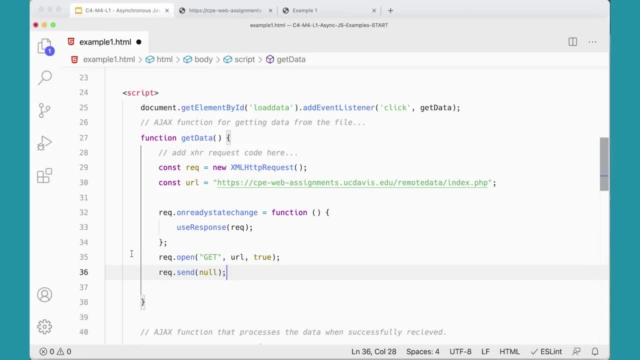 All right, So let's go ahead and add these two pieces here. and the XML HTTP request object has an open method that allows you to say what method in which you want to get that data And what kind of data are you going to send. 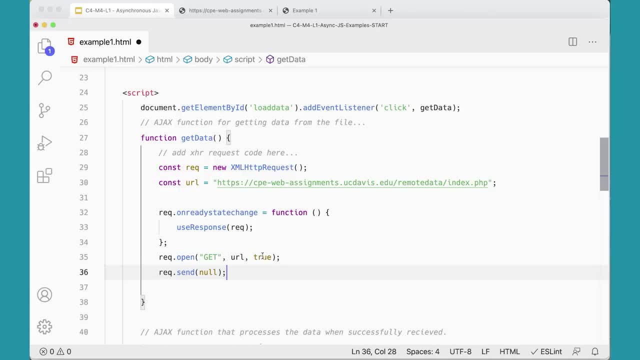 Well, we're sending the URL, that's the data we're getting, and true means do it asynchronously. And then we're also setting the send method to know we're not sending anything back to the server. In this case, we're just getting the data from the server and that's it. 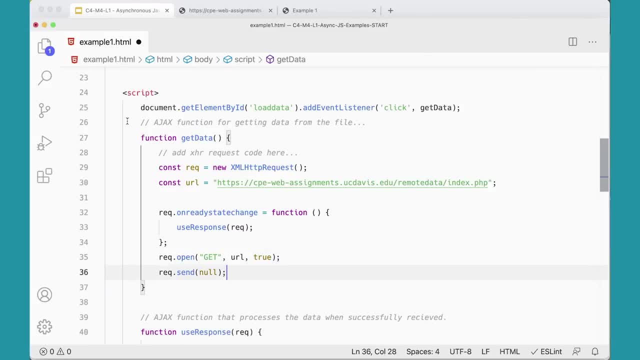 So that's all we need to do with this function for get data Cause this goes and gets the data, waits until the data is ready and then runs this function called user response that will allow us to use that data. Let's take a look at that function next. 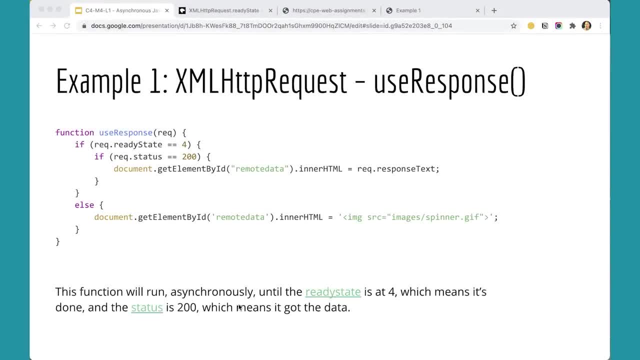 In the last video we built the function that allows us to get the data. Now we need to be able to use the data that comes back, So we're going to have this use response function That's going to check the ready state. 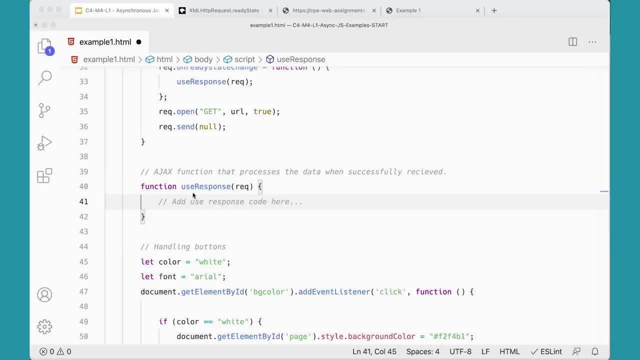 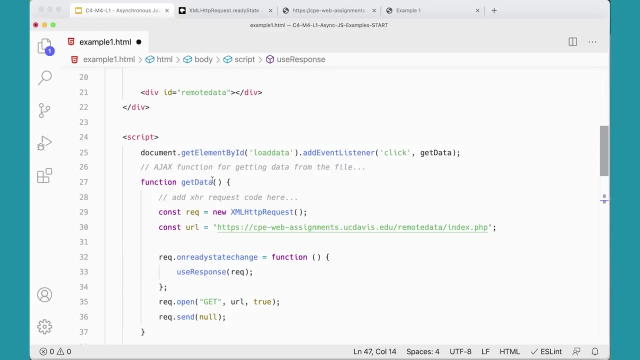 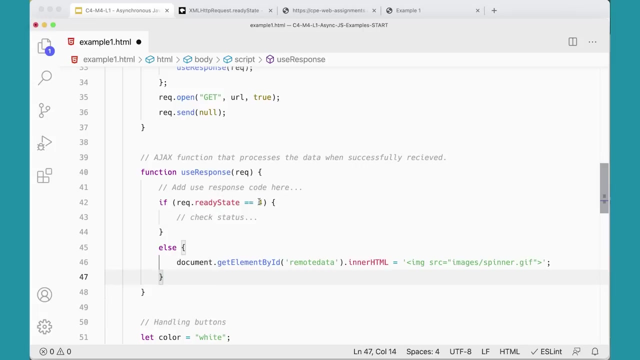 Let's go ahead and build up this function a little bit. Here's the stub for use: response function. here We can add an if statement in. here we're checking the status of our again. this is our XHTML request object. here We're checking it's ready state to see if it's for. and if the ready state is for, we're going to do something else. 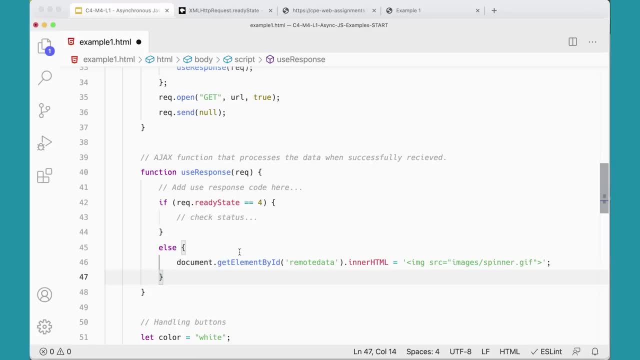 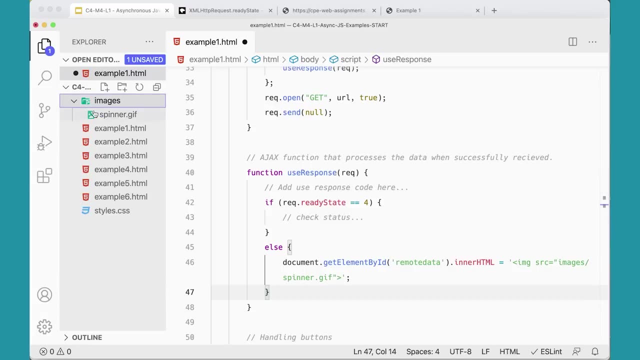 If it's not a four yet, while we're waiting for a four, I've got a little image in my files over here. It's just this little spinner. It's just a animated gif of a spinner that we're going to go ahead and just put on the page. 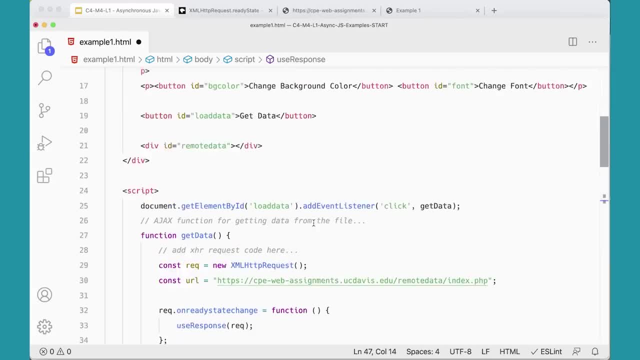 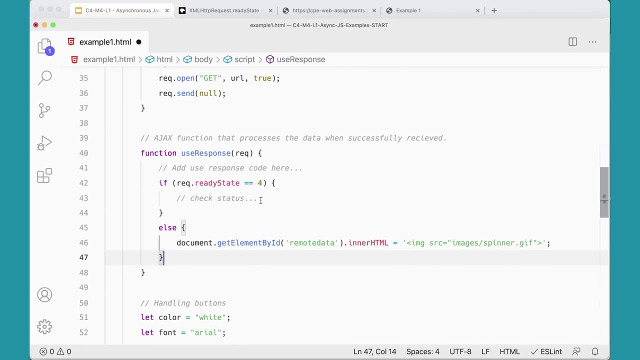 We're going to set that remote data, that get element by ID remote data, which is down here. It's an empty div at the moment. We're going to put a little rotating spinner in there while we're waiting it to be a four. 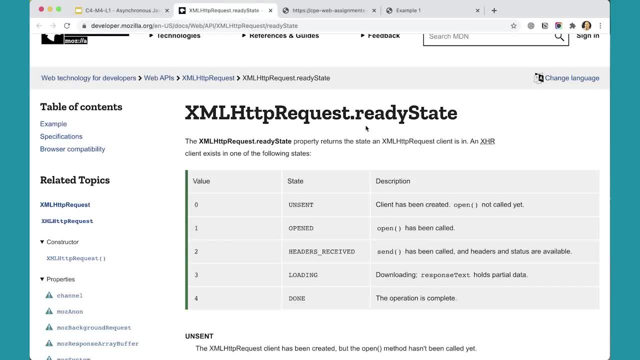 Now, if we come back over here and look at this, the ready state is either a zero, meaning it's been unsent, a one it's been opened, a two- the headers are received. three- it's loading, or four- it's done. 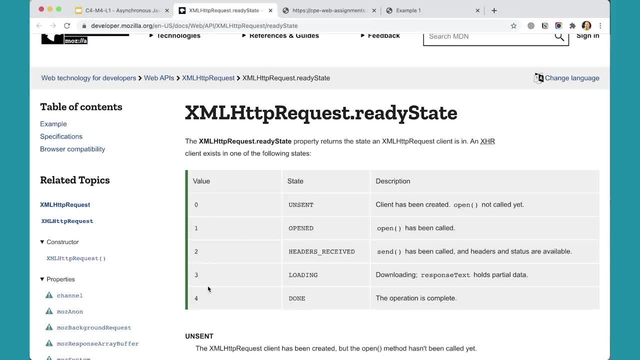 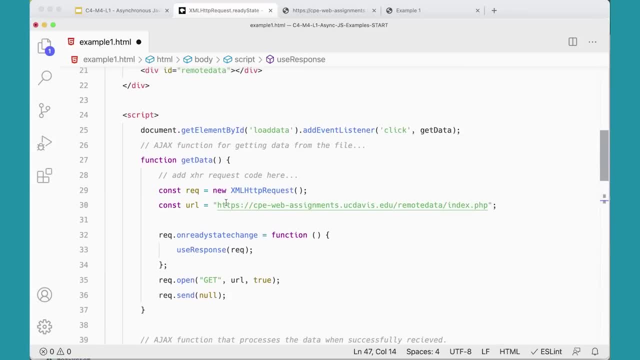 We have the data, the operation is complete, So we're looking for it to be complete And then, if you come back over here And we come back up here and look at this again on ready state change, use response request. So this is going to go from a zero to a one. 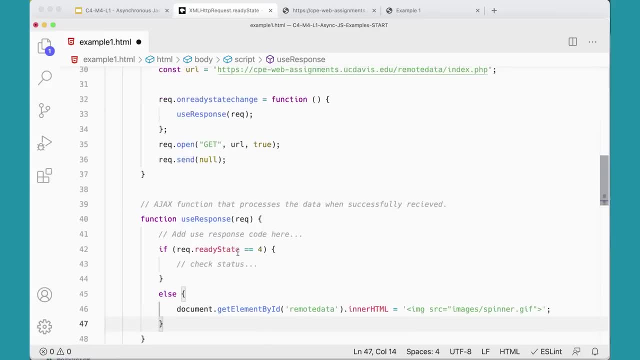 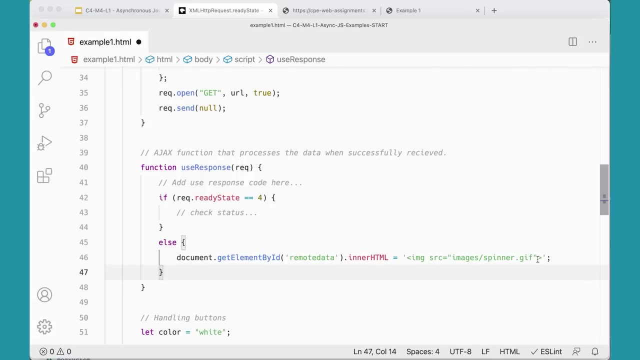 It's going to go through each of these numbers, but it's only until it gets to four that we're actually going to do something. And while it's going through the other things, while we're waiting for it, we're going to show that spinner, if that makes sense. 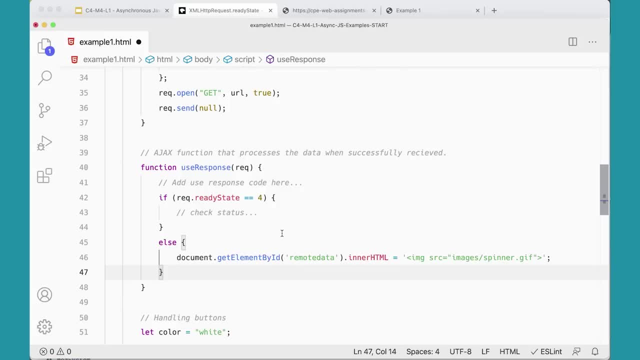 So remember, the page is set automatically to make us wait. It leaves At least five seconds, maybe as many as 30 seconds. Once we have that four and the operation is complete, then we can check the status to see if it's 200.. 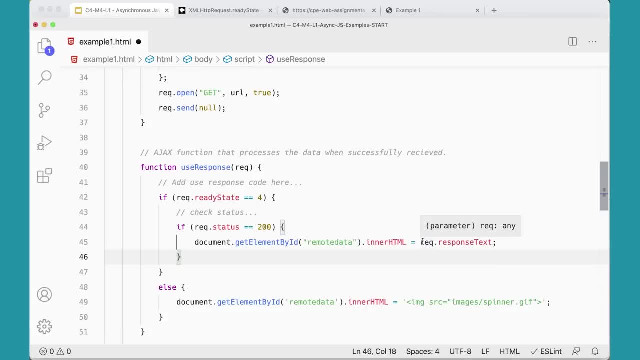 And if it is, then the XHTML HTML HTML HTTP request object has a property called response text And this will actually be our, That we get back from the page. That's the actual data And we're going to go ahead and put that, using inner HTML, into remote data. 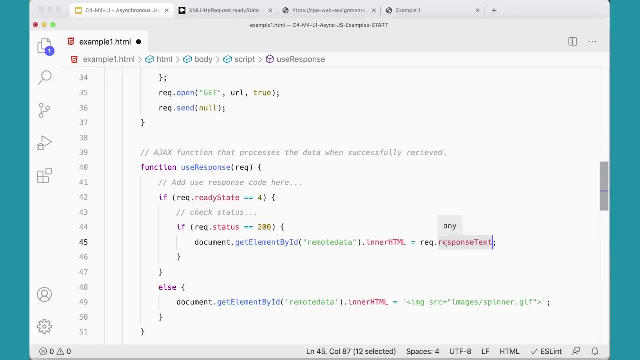 So the spinner gift that was there's going to be replaced with the actual div. Now what does status 200 mean? It means it's okay. It means that it completed the task, It got the page and it's all okay. 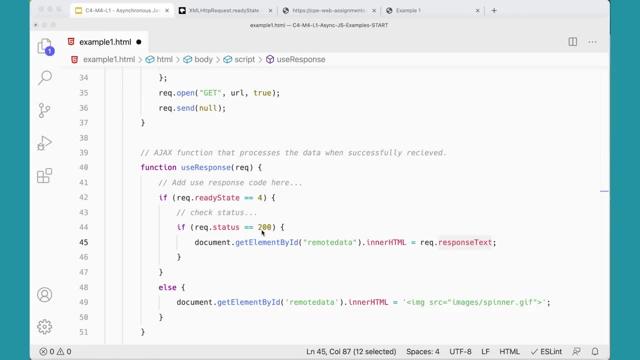 We don't usually see status 200 when we go to websites, but every time you go to a web Page, the server is sending back to the browser a status of 200 saying: okay, I got your page for you, It's done. 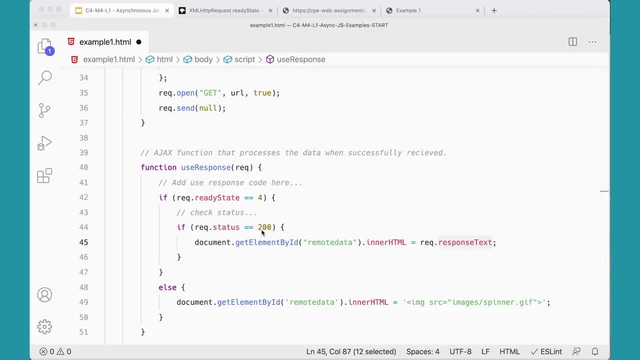 Here it is: If you don't get the page, if there was some sort of- if you requested URL that didn't exist, you'll get a four or four, And sometimes you see those statuses. You'll get a page that says four or four not found, or sometimes, if there's a server area, you'll get something like a status 500. 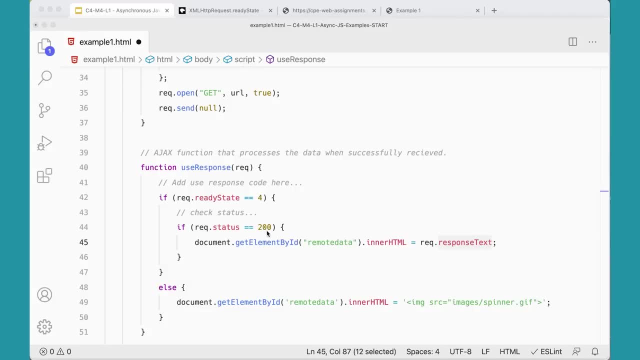 So there are different status numbers to Indicate what happened with that request and 200.. You never see, but it happens every time. you request something and you get it and it's fine. So, um, we're looking for that status 200 and then, if we can, we're going to, if, if that comes up, that's great. 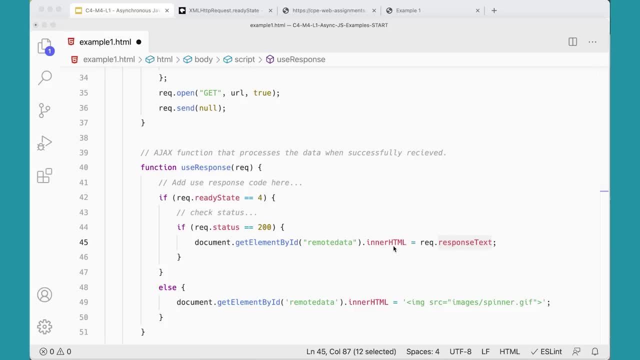 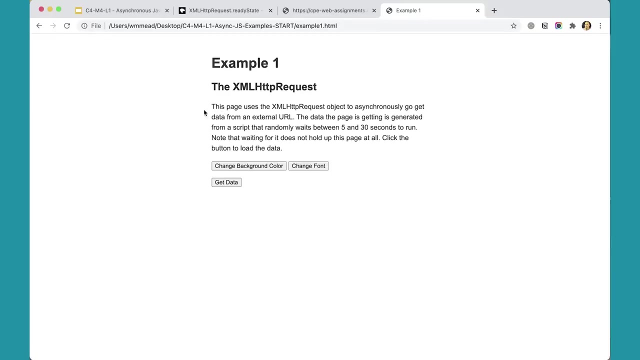 That means we've got our text from our page and we can go ahead and put it on our page. That should be all good. We can save this, And then I should be able to come and test out my example here, and while it's running we can click the get data button. 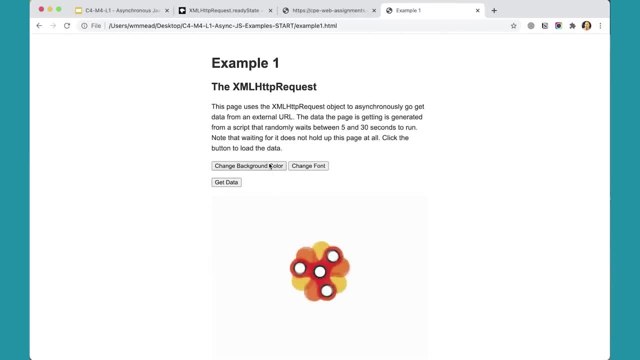 And while we're waiting for that data, however long it's going to take, we can interact with the page. We can change the background color, We can change the font. We were not being Prevented from doing these other actions on the page while this thing is going and getting this data. 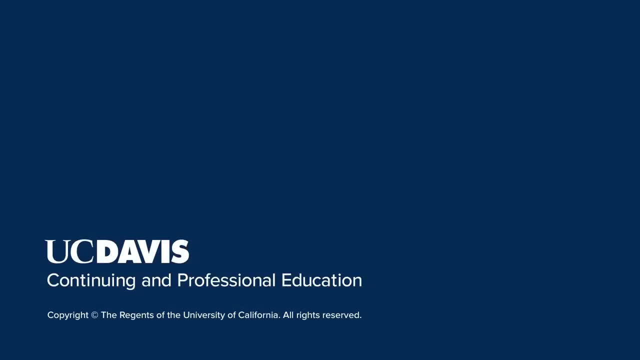 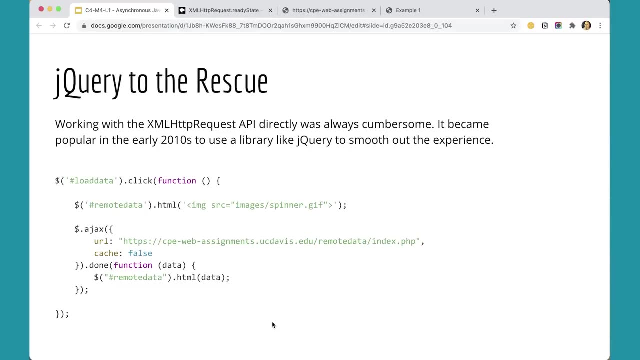 And that's asynchronous. Jay query to the rescue. working with the XML HTTP request API directly was always cumbersome- kind of like the name- but it became popular in the Early two thousand tens to use a library like jQuery to smooth out the experience. 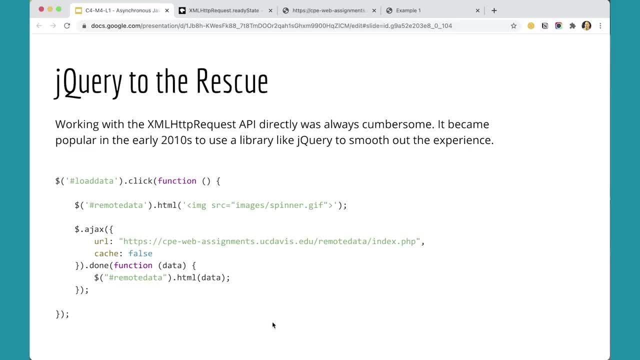 And there are other libraries that have been dedicated specifically to working with the XML HTTP request API and smoothing it out. But all of these libraries are really just using that XML HTTP request API. It's just they've kind of tucked it away and hidden away and make it made it a little bit easier to use. 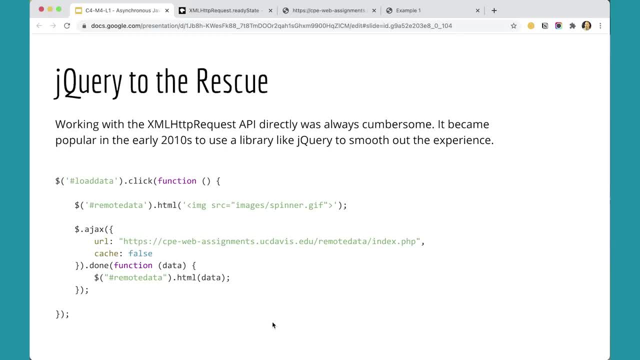 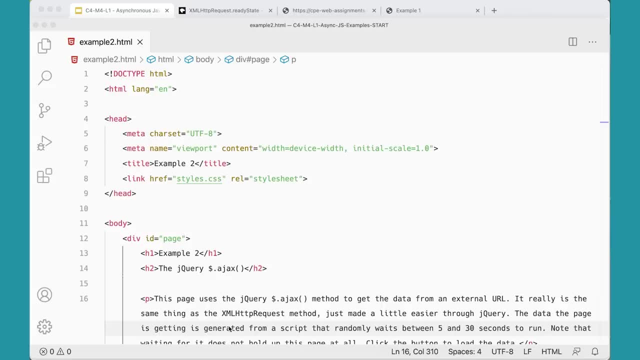 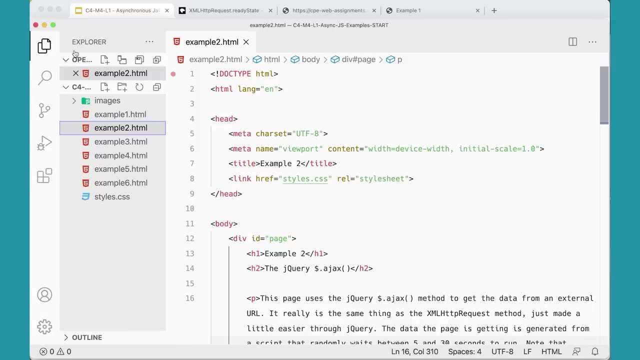 So let's take a look at example two, Because example two will use jQuery to do the same thing that we did in example one. Here I am in my code editor looking at the example two file in my examples over here. I just got the Explorer closed so it doesn't take up room on the screen. 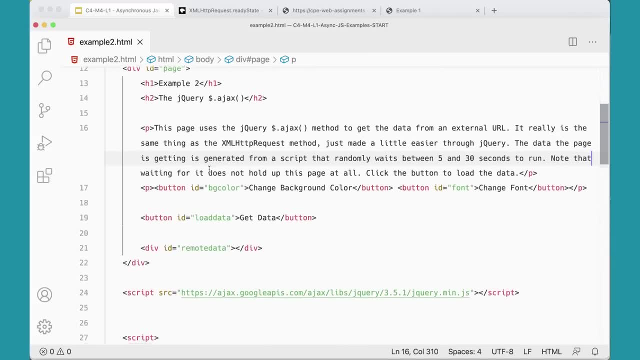 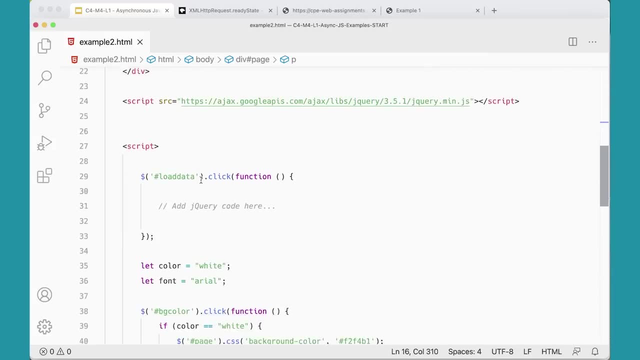 And here we've got example two, and it's using the jQuery version. here and down here I've got the exact same div- remote data- that's empty, that we're going to load our data into when we have it. And then down here I have a script with a click handler that's looking for a click. 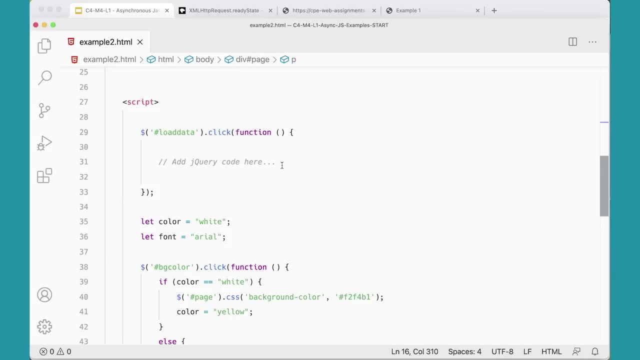 It's going to run this anonymous function and we can actually add our jQuery in here, And the first thing I'm going to do is go and get that remote data div and stick the spinner in there. So the spinner goes in there, no matter what. 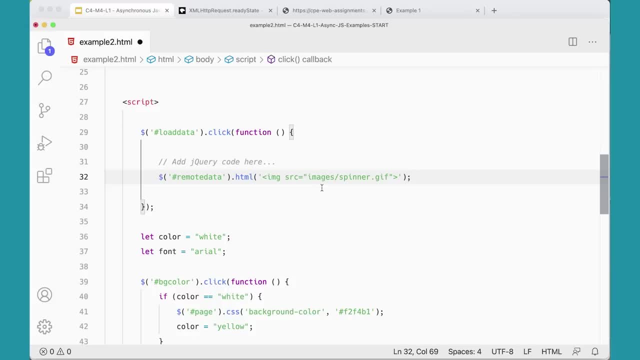 And then we're going to add our Ajax method to go and get the data from the server And that looks like this: $ajax. Okay, so this is the Ajax method in jQuery, And remember, the $ is just short for jQuery, So this is just really the same as jQueryajax. 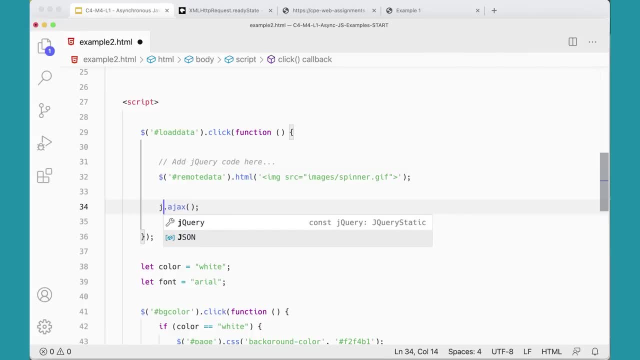 jQuery do your Ajax method. So it looks a little weird because of the $, But it's the jQuery method, Ajax- And then we're going to pass in an object here And in the object we're going to put a few members of this object. 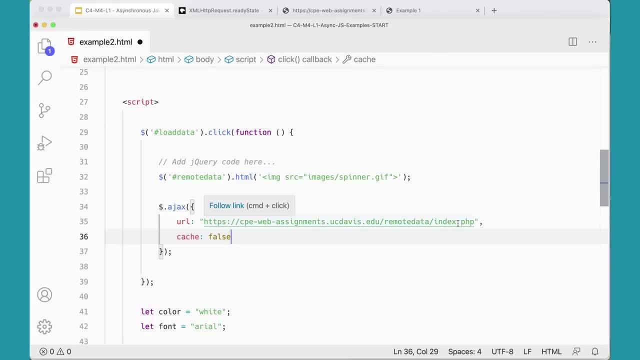 The URL, which is the exact same URL we were using before, And cache false. So that means get it every time, Don't let it get cached, So that's going to go out to the server And then we're going to pass in this URL and get that data. 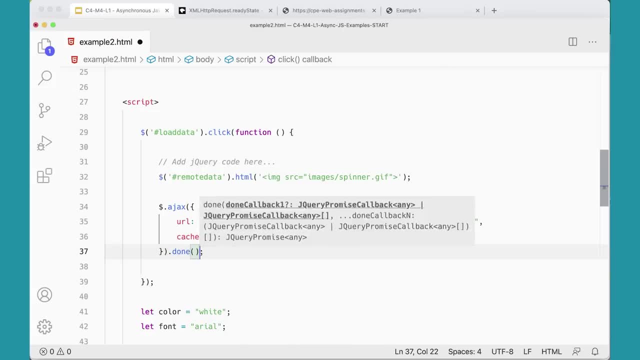 And then we're going to chain a method at the end called done. That's going to run when this thing has successfully completed. When it's done, we're going to run an anonymous function. That's going to run when it's done. 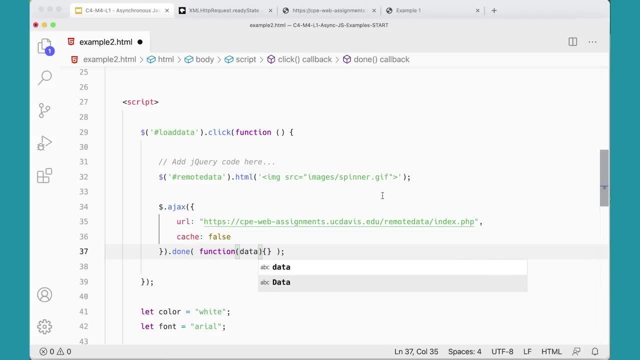 We're going to pass into this function the data that comes back from this request. And what do we do with that data? We're going to basically do this. I'm just going to copy that and stick it down here. But instead of sticking in the spinner, we're going to stick in the data. 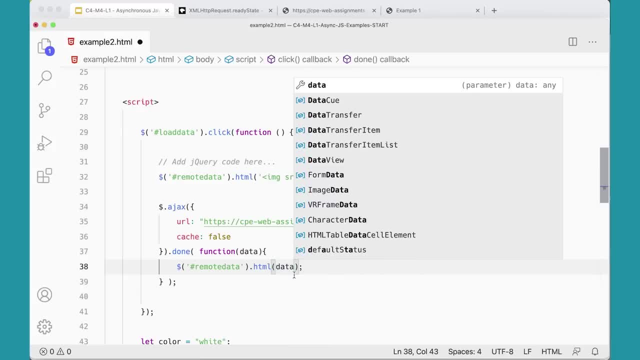 So that will be our div, that we're getting from our page, And that's it. That's all we really need to do with jQuery. So jQuery, the syntax is a little bit simpler. It's a little bit more straightforward, A little bit easier to use. 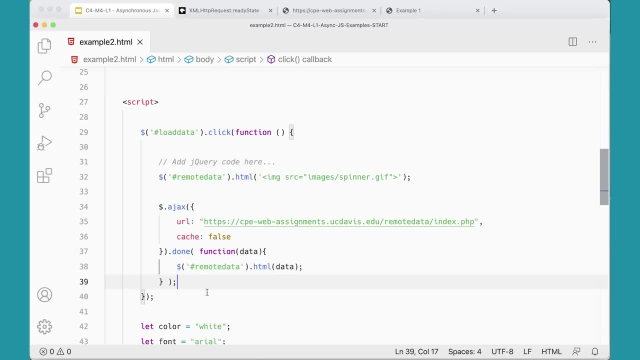 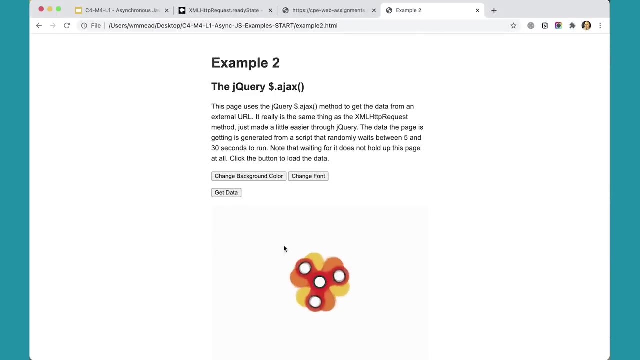 The XML HTTP request thing is not such a mouthful. We can just use AJAX, which is kind of nice. Let's see if it works Here. I am on the example 2 page And I can click get data. And I've got my spinner. 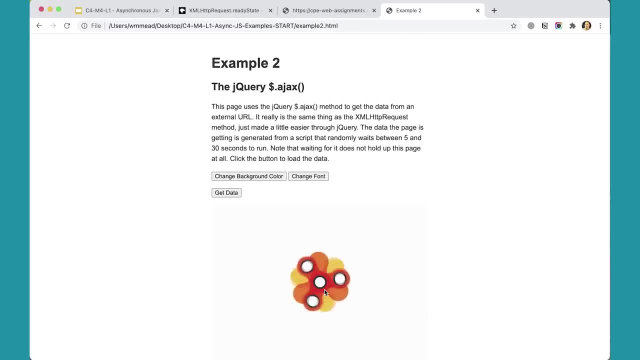 So it's gotten that This is just an animated GIF. It's not any kind of fancy animation or anything, But it's just an animated GIF. So it's running that while it's going off to the server And waiting for that server. 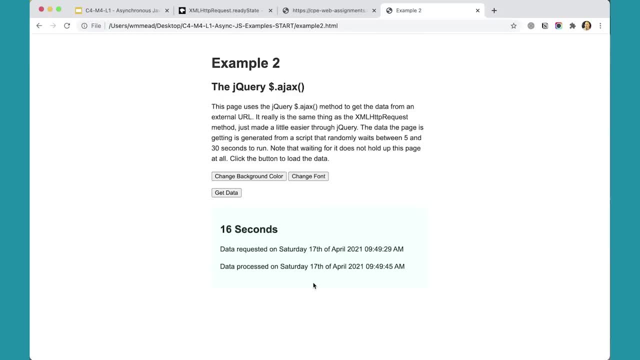 To process that request, Which will take between 5 and 30 seconds, And it took 16 seconds. The other thing is that while this is doing this, We're not blocked from doing other things, So I can change the background color. 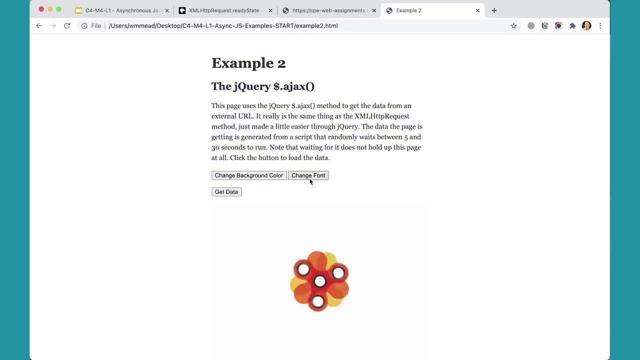 I can change the font on the page. That's what the rest of that JavaScript was on the example file over there. I didn't really talk about that, But that's stuff that we've done before, So we can change these things. It will run those click handlers. 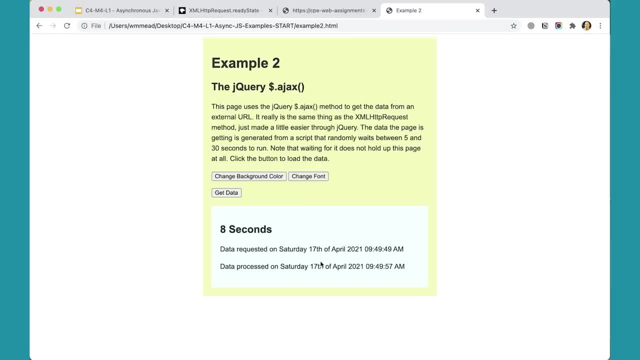 While it's waiting for this to come back. That's just sort of put on hold. It's just waiting for that to get its response And waiting for it to get to that 4 level And the 200 status so that it's done and can be displayed on the page. 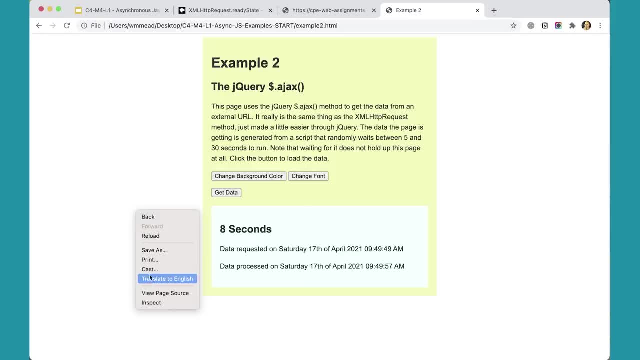 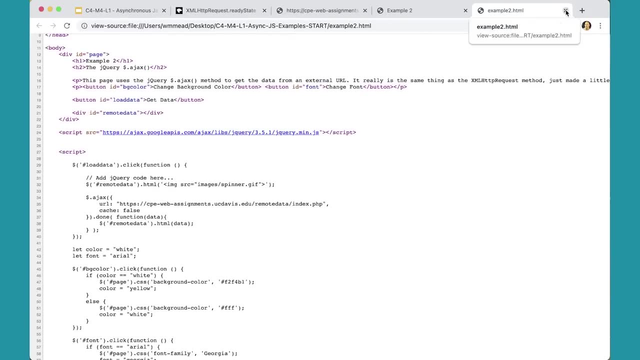 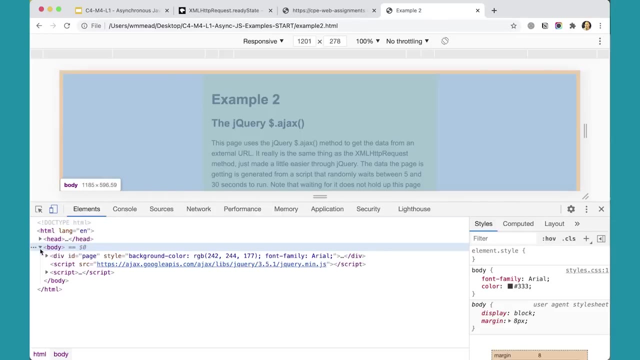 And then we're just getting that div and filling it in. If you were to view page source here, You would see nothing. This is empty here. But if I were to inspect, You would see. If I drill Down here in my HTML, 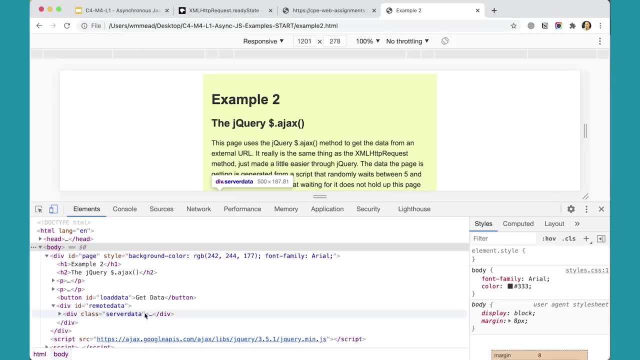 You'll see this remote data div has now got a div class server data in it. That's come over from the server, that Ajax appended to the page there For however long it was going to take for it to complete, And that's really pretty cool. 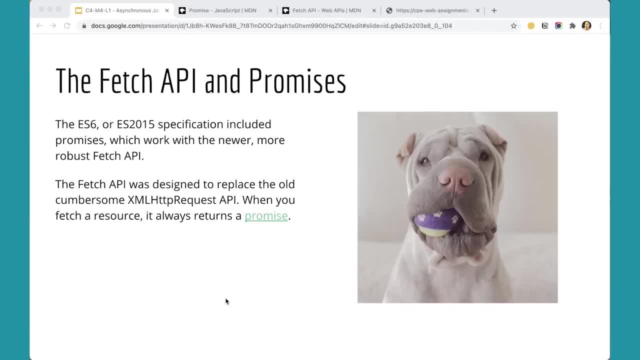 We have the old XHTML HTTP request API And it still works and you can use it. And it's a little bit cumbersome to use in playing vanilla JavaScript, But it's certainly doable. And then on top of that there are libraries like jQuery and other libraries that also make use of that API to do asynchronous requests for JavaScript. 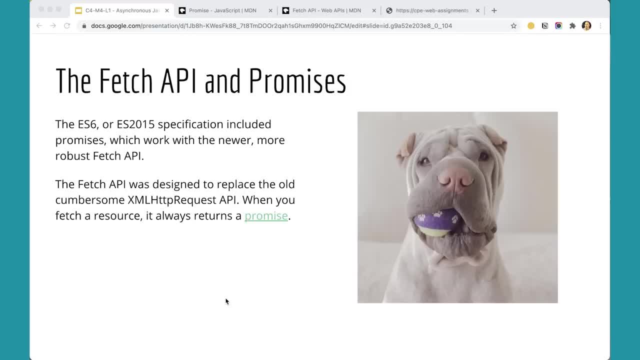 However, the JavaScript world is moving on And the fetch API And promises is the future for asynchronous work with JavaScript. The ES6 or ES2015 specification included promises which work with the newer and more robust fetch API. The fetch API was designed to replace the old, cumbersome XHTML HTTP request API. 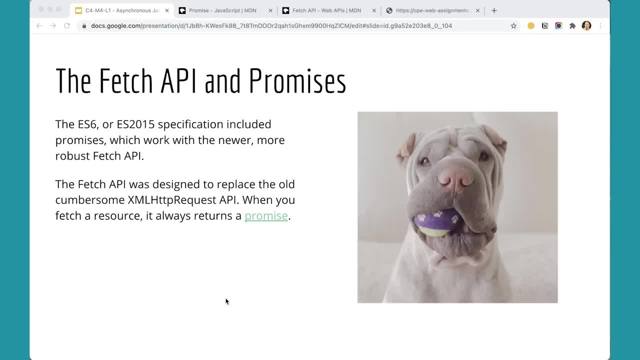 When you fetch a resource, it always returns a promise. A promise is resolved And is always in one of three states. pending fulfilled or rejected Promises. use the then method to handle data when the promise is fulfilled. So we'll take a look at example three in the next slide. 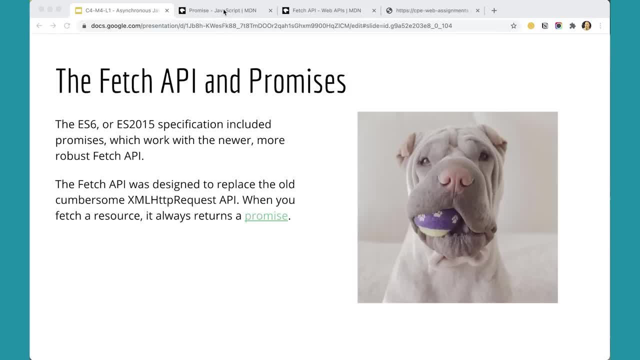 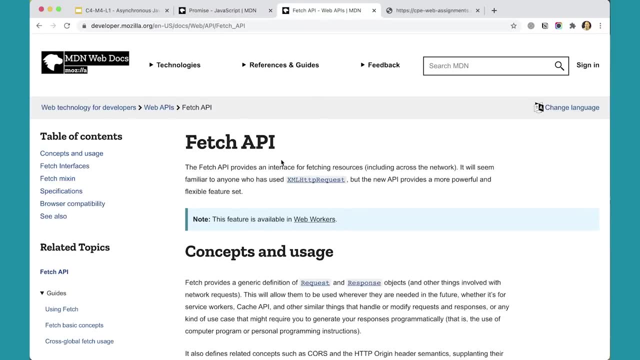 Before we do, I recommend going over to the MDN and looking up promises and fetch API and reading up about it. It's kind of techie and a little bit more complicated than what you'll get from this lesson, But I think for more in-depth understanding it's really helpful to know more about these APIs and how they actually are designed to work. 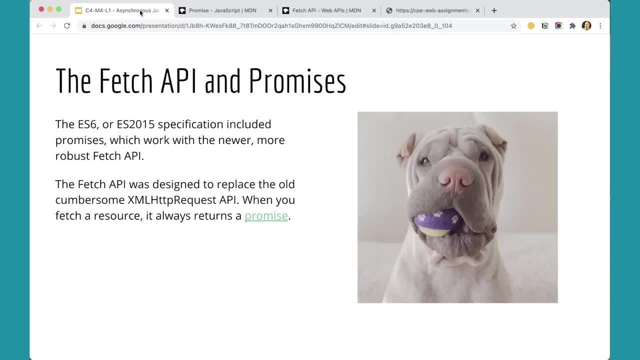 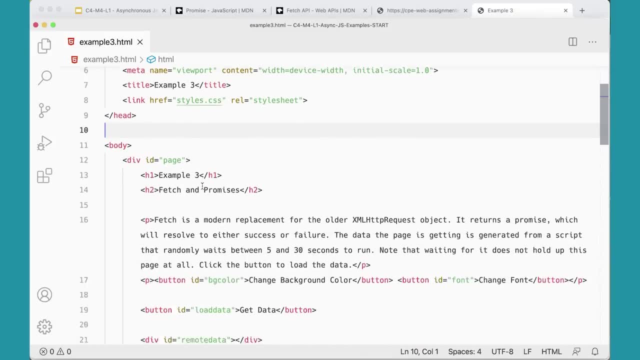 And get into it a little bit more deeply than what I will show here. If you look at the code, for example three, you'll notice it looks very similar to what we had before, Except now we're going to use fetch and promises to do the same thing. 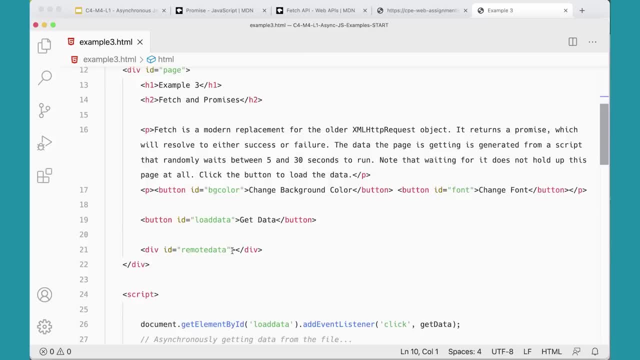 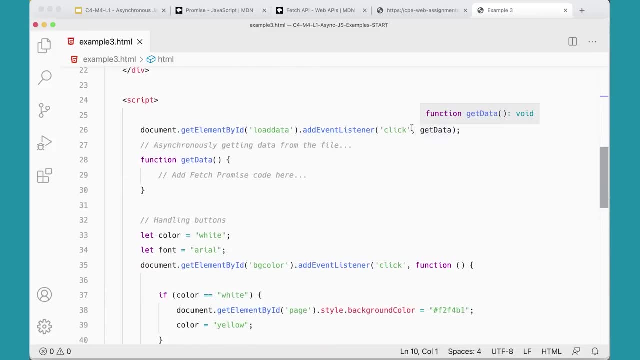 We've got the button to load the data. We've got an empty div for the remote data when it comes in, and down here I've got an event listener listening for a click when you click that button to load data and then it's going to run this function, get data here, and this is where we're going to add our code down here. 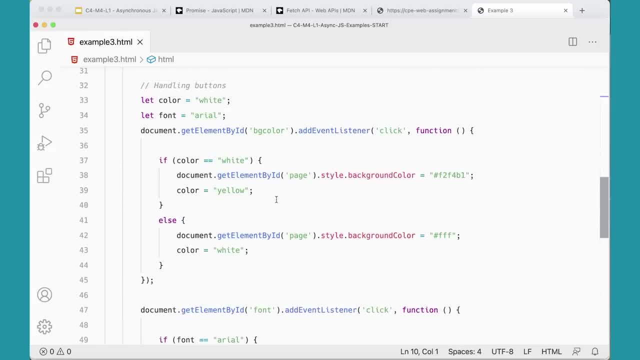 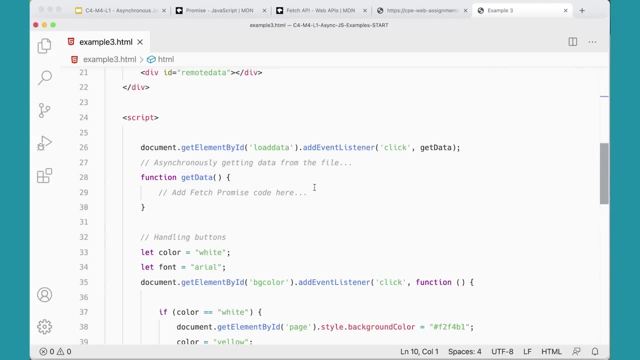 We have our methods for switching the fonts and the colors that we had before, So there's nothing fancy going on there, but this is the function that's going to get the data, And so let's go ahead And add some stuff in here. 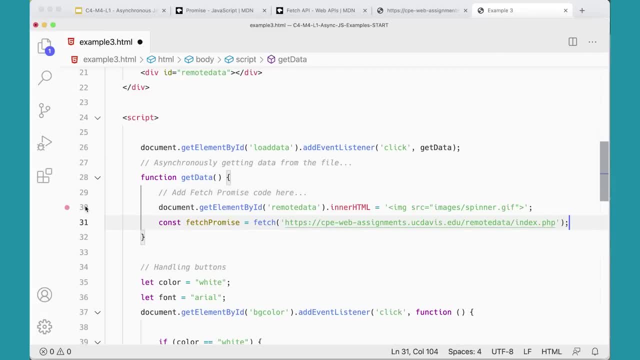 First, we're going to do exactly the same thing that we did in the jQuery version of the project, where we just go and get this element by ID and set its inner HTML to the spinner gif, And then we're going to make a variable called- and I'm just going to call it- fetch promise. 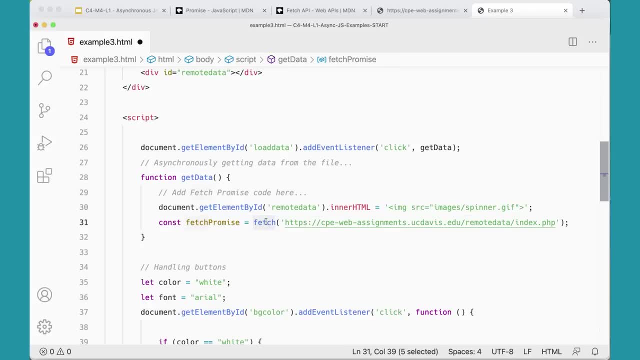 You could call this variable anything you want, but it's using this new fetch API and I just give it the URL, which is the same URL We've been using all along, and that's going to go and get the data and stick it into this fetch data, fetch promise thing here, into this variable. 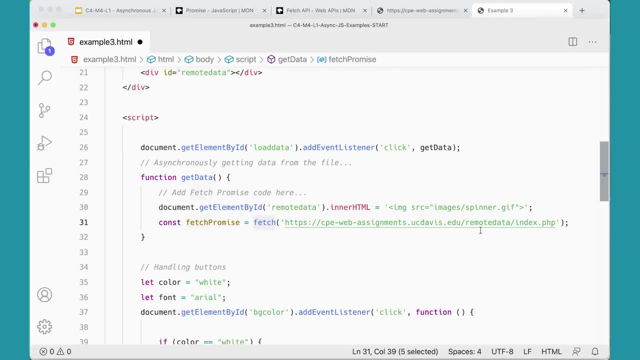 But this variable is going to actually hold this whole fetch API and its results and all that stuff. It's going to be inside fetch promise and this is going to be a promise. This is actually going to be a promise because we're using fetch and fetch gives us a promise and a promise is either resolved or not resolved. 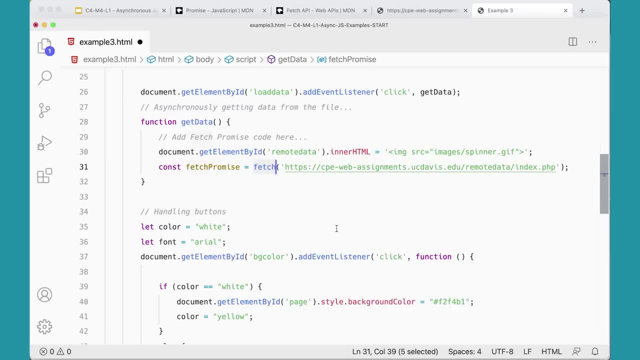 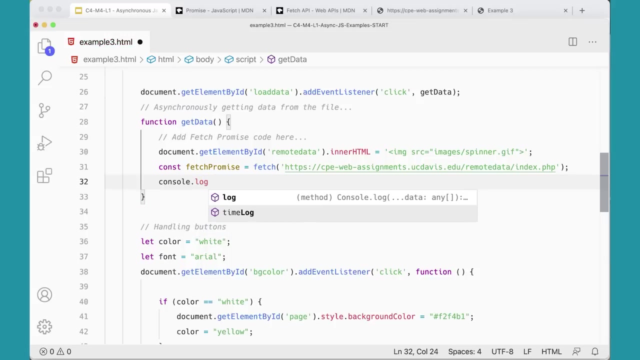 And it's either successful or it fails when it gets resolved. Okay, so we've got all of that And, honestly, if this promise thing seems a little vague to you, we could consolelog out fetch promise to see what's actually in there. 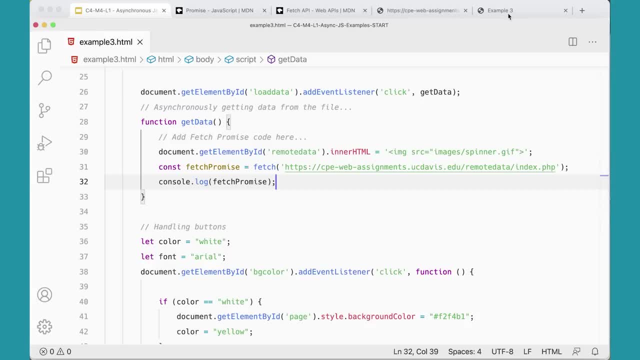 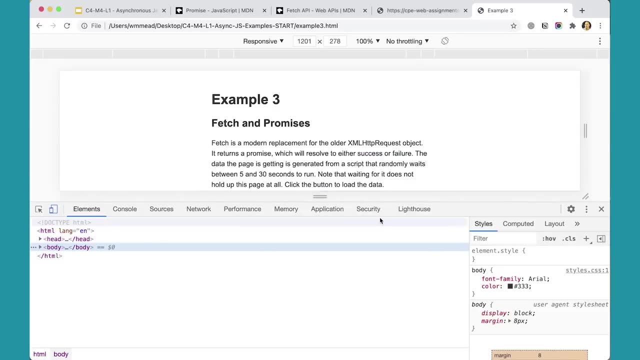 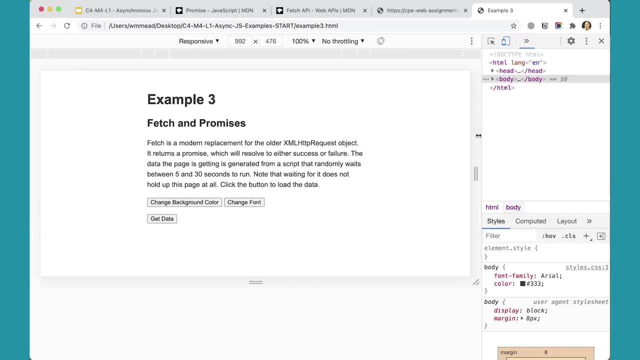 So let's just do that, just to see for a second what's going on over here. So if I go to example three, I'm going to inspect And turn on my, I'm going to move this so that it's on the right side there. 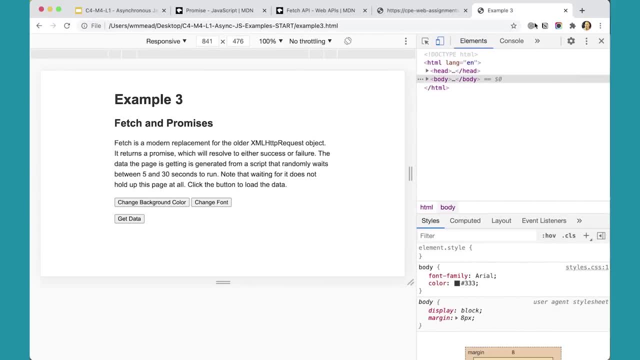 Maybe make it a little bit wider and go to my console And then, when I click get data, I may have to refresh here Get data. You can see that I've got a promise and it's pending. I don't know what's going to happen with it yet. 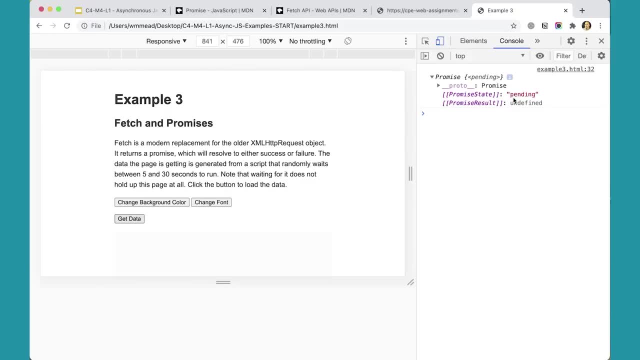 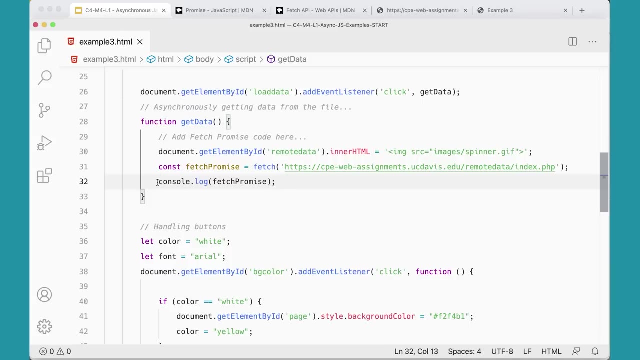 But that thing is a promise And the state is pending, So that's kind of what is going to be held by that variable at this point in time. Great, Now that I know what that does, I can take this thing out. I don't really need it. 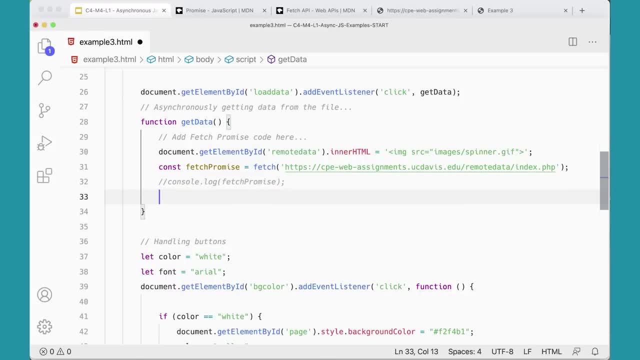 But it's fetch promise holds a promise, And I need to do something when that promise is either rejected or when it fails, or when it fails Or when it's completed. So I'm going to use fetch promise dot then And I'm going to chain this then method on here. 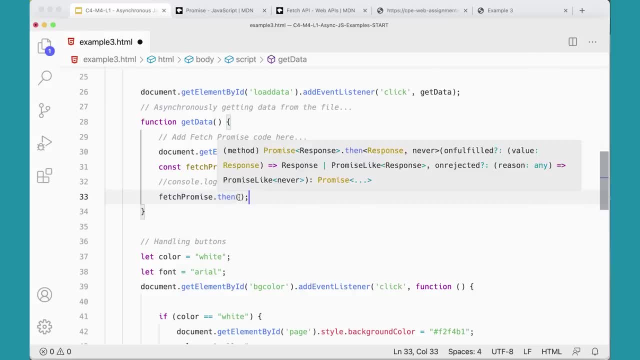 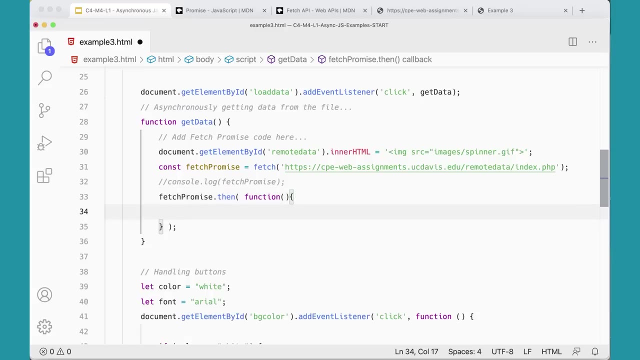 Which is going to handle what happens when the fetch promise completes. I'm going to pass into this a function, Just a normal function, Oops function With curly braces, like so, Like that. This function is going to get the text that when the promise is resolved, 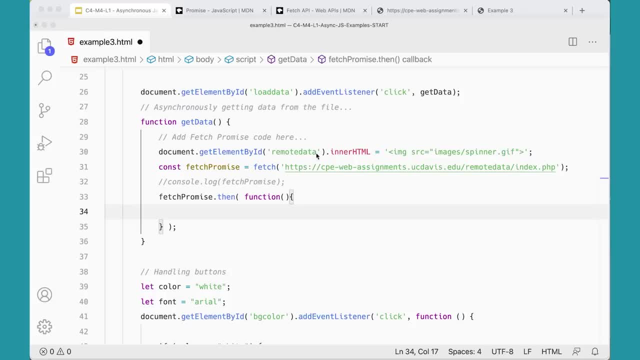 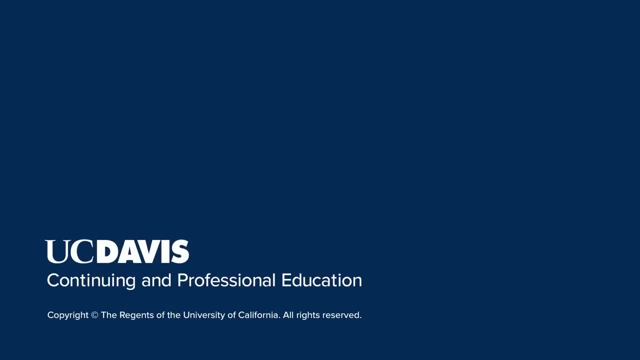 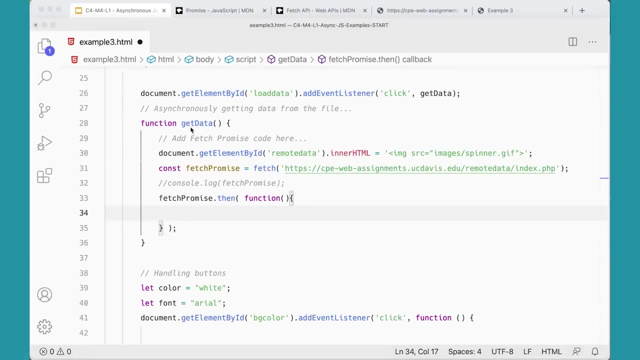 And then put it back into this inner HTML for remote data, And we'll do that in the next video. In the last video we started setting up our get data function to asynchronously get the data from our server. We have our spinner on the page. 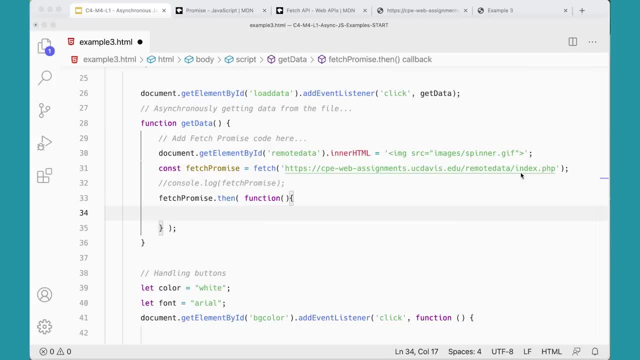 We've gone and fetched the remote URL And then we've taken that variable that has that promise in it And we have used the then method to run a function. And in this function we're going to pass in a response object And this response object is going to get resolved to hold the function. 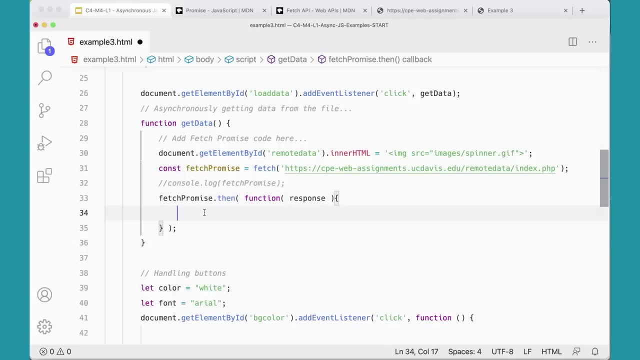 To hold the information that we need to get back, And I can see that if I console log in here: responsetxt. So let's just see what this does really quickly, Just to see what this response thing has in it. So I'm going to come back to my example 3 here. 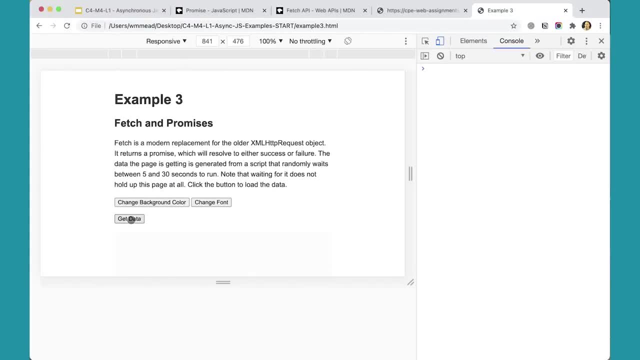 Refresh the page And if I click get data, you'll see that it appears to be doing nothing until I actually get some response from it. Hopefully that will take- not 30 seconds in this case, But we shall see. Okay, you can see that it finished. 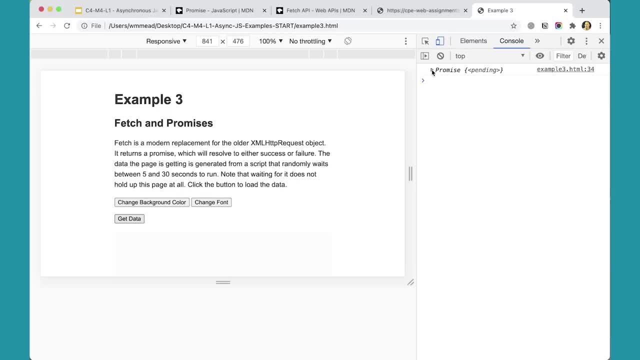 And I have promise pending here And then if I open that up, it says: oh, look at that Promise state fulfilled. And then in here the promise. I've got an object called promise. result: that has my div class server data. 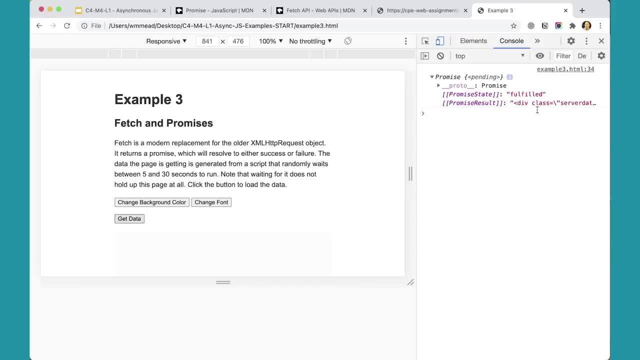 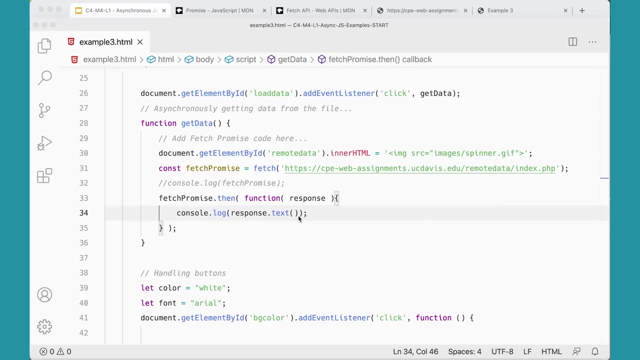 Has the data coming in from that actual, From the actual server. So that's what's being held in that. in that object, The response object is holding these things about the promise itself, including the actual data. So that's working. So we know that response text has their actual data in it. 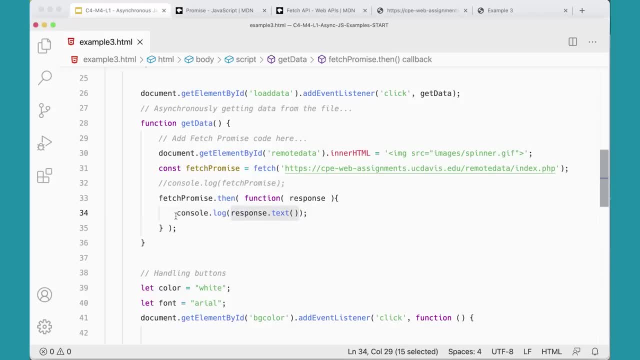 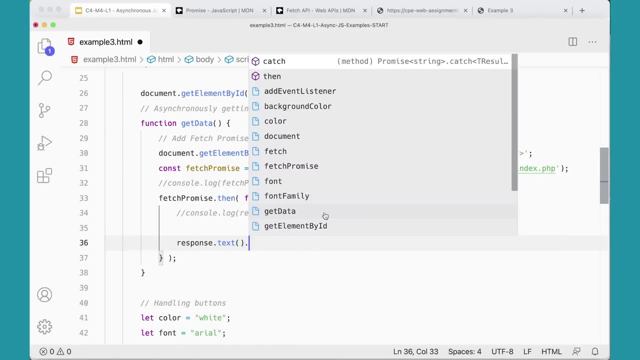 So we could take that out of here. I'm just going to comment that out because I don't really need that, But I can take that and I can say I'm going to chain another. then on here, that's going to run, And in here is yet another anonymous function that's going to go function. 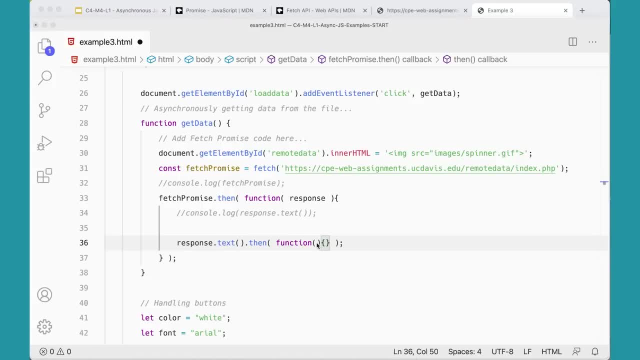 Like so, And I'm going to pass into this function the actual text of this response here, The response text. I'm going to pass that in And then in here inside these curly braces, I can just go to my document, get on by remote data and put the text on the page. 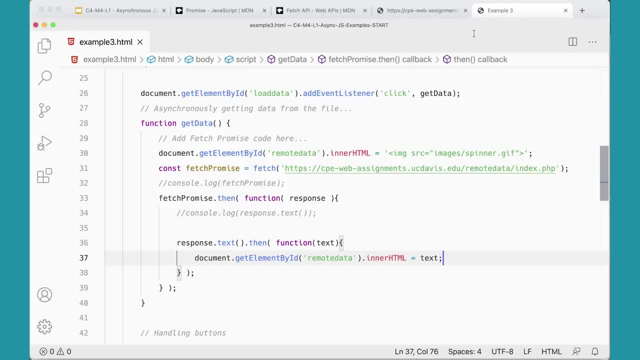 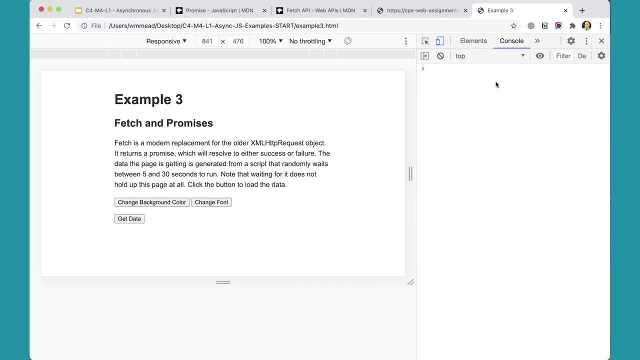 That's kind of a long one, But let's go over and test it out and see if it works. If I come over here to my page and click refresh And then if I click get data, I'm going to turn off my inspector here. 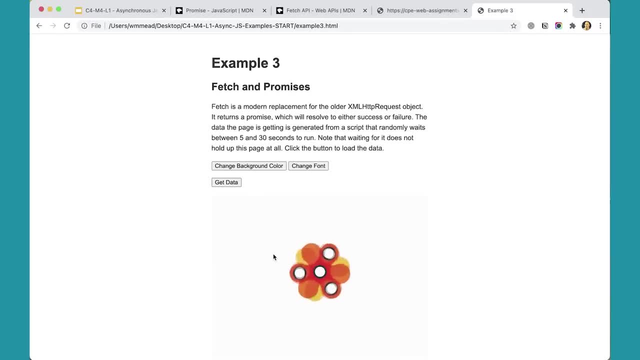 Click get data And you can see it's running. My spinner got loaded, It's doing its thing And it's going and trying to fulfill that promise. While it's doing that, I'm not blocked from doing anything. I can change the font on my page. 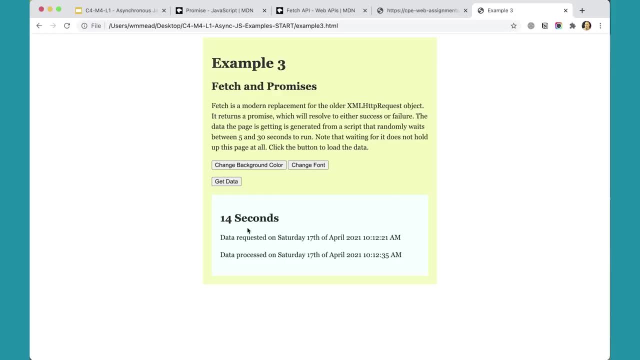 I can change the background color and do all that stuff. And it took 14 seconds to complete and go and get that data And then when it returned it, it put it in the page. Now, if this then chaining thing seems kind of complicated, it is. 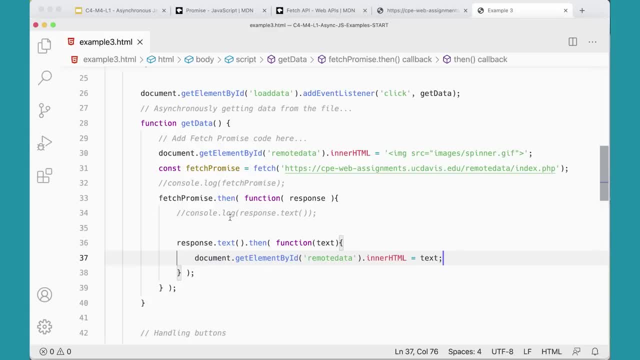 And we've got a solution for that that we'll look at next. But what we have here is actually not that different than what we did with the jQuery version. It's a little bit different, but it's not that different. We put the spinner on the page. 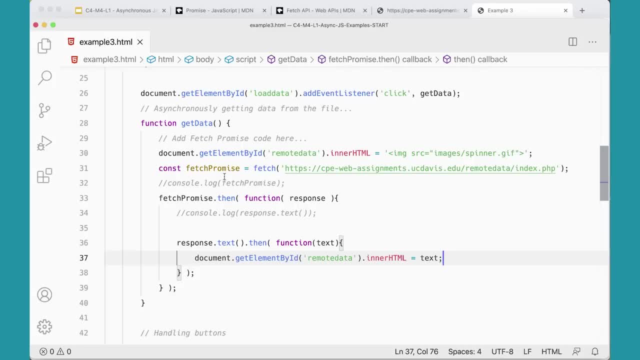 We go, instead of using the jQuery AJAX API, we've got the Fetch API And we're passing in the link that we're going to And that gets put in a promise, And when that thing is resolved then we can do something with it. 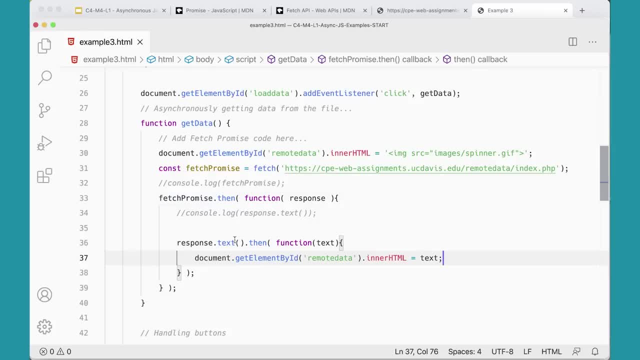 And it really is fairly simple. It just feels a little bit complicated Because we've got two of these then statements that we're chaining in here to kind of figure out how this is all going to work with two anonymous functions, And we're going to take a look at a way of making that a little bit simpler in the next example. 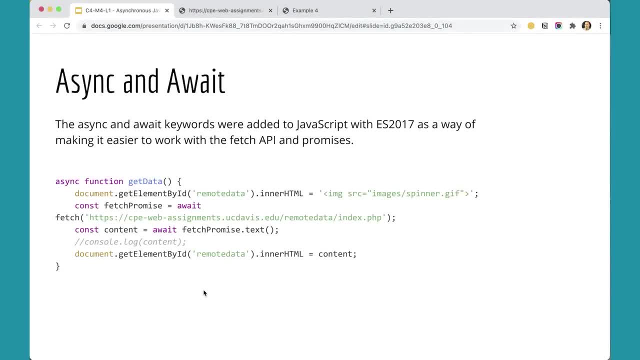 Async and await. The async and await keywords were added to this. We added to JavaScript the ES2017 version as a way of making it easier to work with the Fetch API and promises. Because of all that chaining of the then stuff, it just got to be kind of complicated. 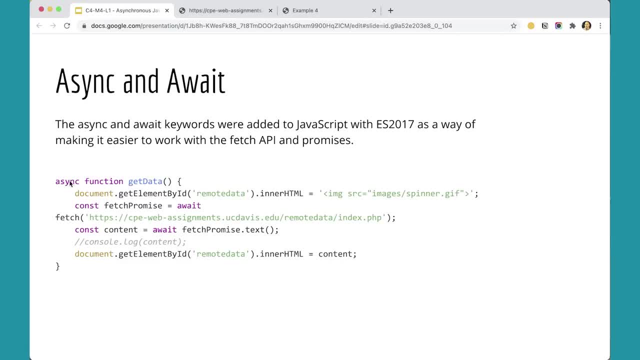 So here you can see, we have a function here, but it's got this async keyword in front of it, And then we have an await down here that will help us with the async function. So let's go ahead and take a look at how this works. 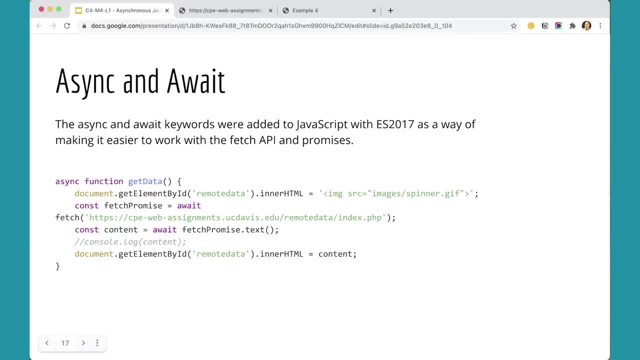 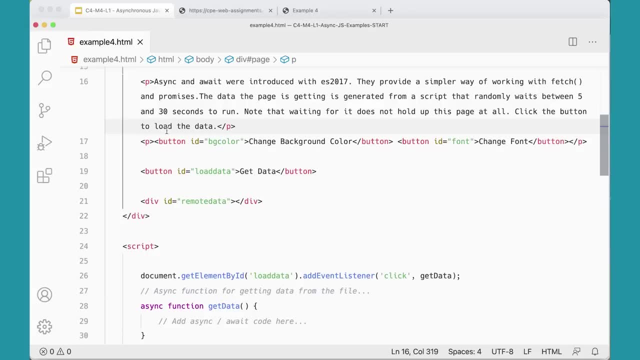 And take a look at this example. If you come over to our code editor here, I have example 4.. And most of the page is not changed. I still have a button for load data. I still have a div for that remote data when it comes in. 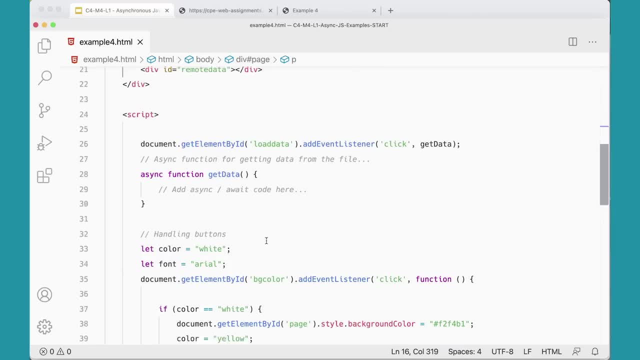 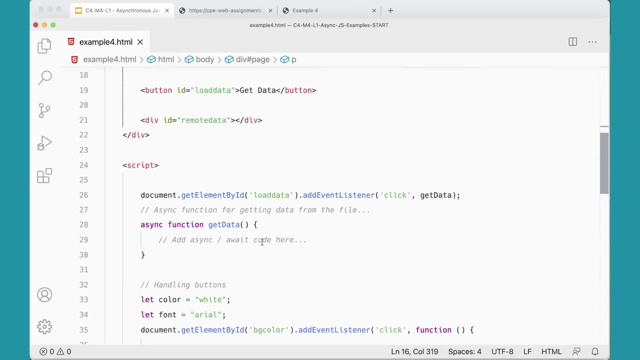 This is where we're going to do our work in here, And then down here I've got the buttons for handling the color change and the change of font, Just so we can click on those and see what happens with that stuff. But here we're going to do our work in here. 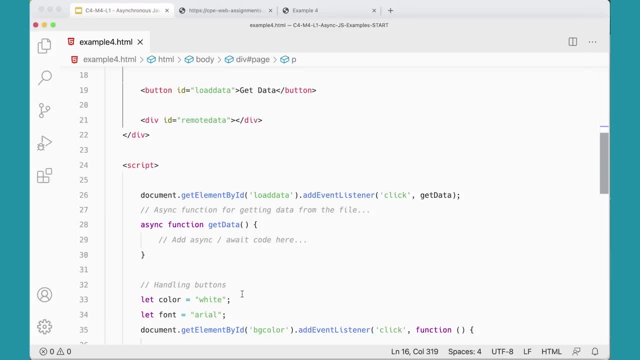 But here we're going to add some code for our async thing. Now notice, I've got the async keyword before function here. It's a keyword that allows JavaScript to know that this function is going to run asynchronously. Let's start adding to this. 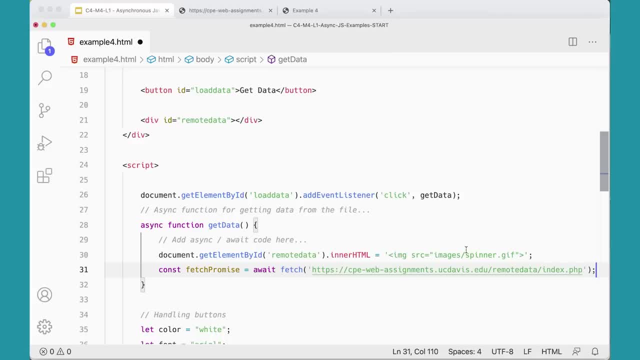 First, as before, all we're doing is sticking our image with our spinner on the page, No big deal. Then I have a variable fetch promise. Same variable as before, And the difference here is I'm putting await before the word fetch. 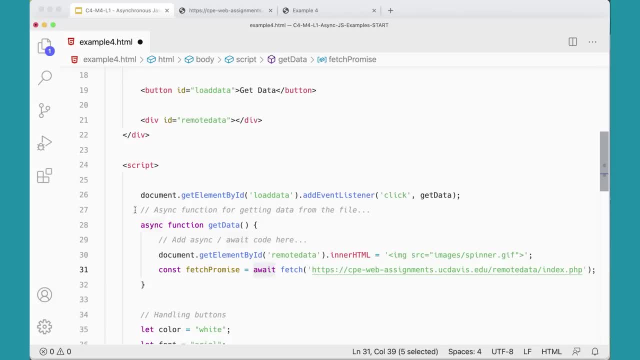 The only time you can use the await keyword is on a function that has async in front of it, So these two things have to go together. If I were to remove async from here, the await would not work, So this is going to just wait for this thing to return its data. 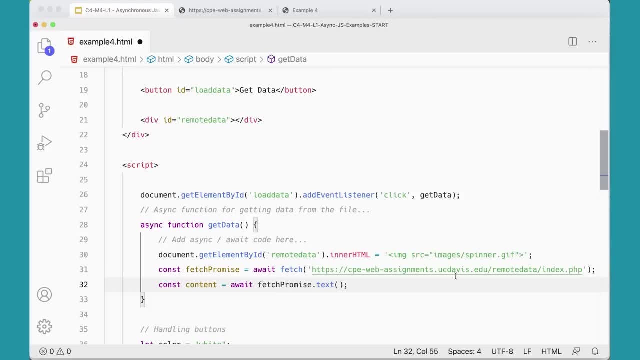 And then I'm going to set up a variable here- My content- And it's awaiting for that fetch promise text. So this is just going to wait for that fetch promise text to come back And I can again use this await keyword, because this is an asynchronous function. 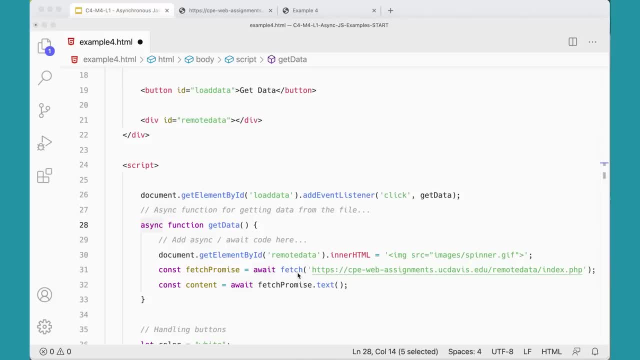 The text method here is going to return the actual text that comes back from this URL. So content is going to hold the actual text once the promise has been successfully completed. And we're still working with promises. It's just that we're using async and await rather than the then method for accessing that content. 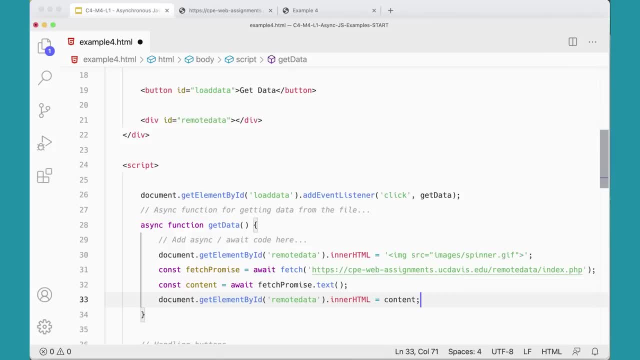 So now I can just take content and I can just put it inside my inner HTML And that's all there is to it. So this is four lines of code. really, That's not so bad, That's actually fairly simple. Four lines of code. 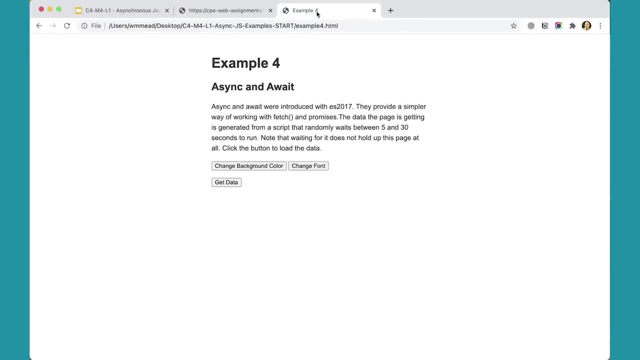 Let's save it and test it and see if it works. If I come over here I'm going to refresh this page. If I click get data, I've got my spinner. It's going to take between 5 and 30 seconds for that to complete. 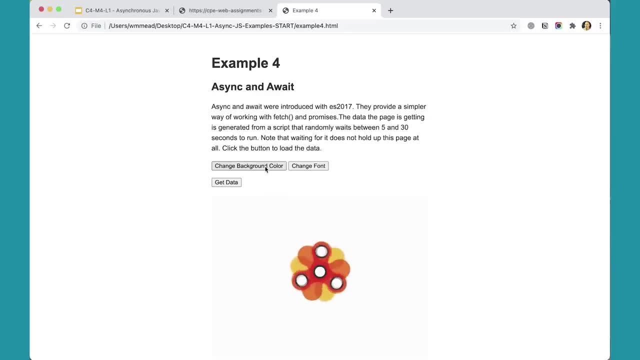 While that's going, my page is not blocked because JavaScript has sort of put it to the side. It's waiting for it to end And I can change the color, I can change the font and do all that stuff. If we go back to the kitchen metaphor, I could be while my eggs are cooking. I could be pouring my glass of orange juice. 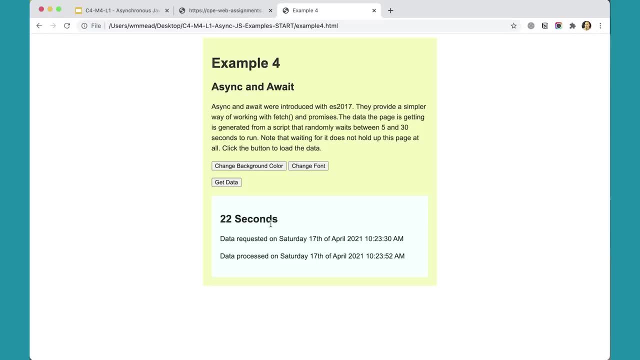 And however long that takes, it takes And when it's done, it says okay, I'm done, And it returns 22 seconds and says that's what it actually finished And that's how long it took to actually complete that one. in that case, 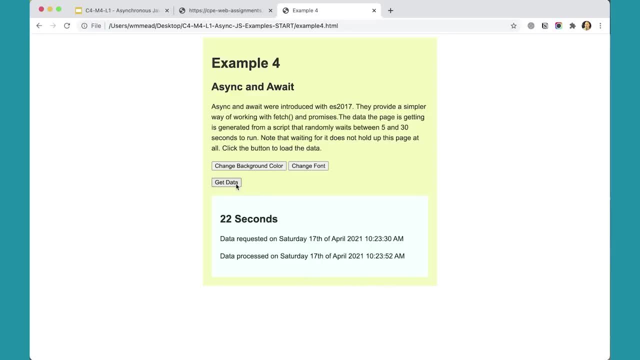 If I were to get data again, it would take a different amount of time- between 5 and 30 seconds- But the page is not blocked, which is really pretty cool. I recommend looking up async and await on the MDN and reading about them there. 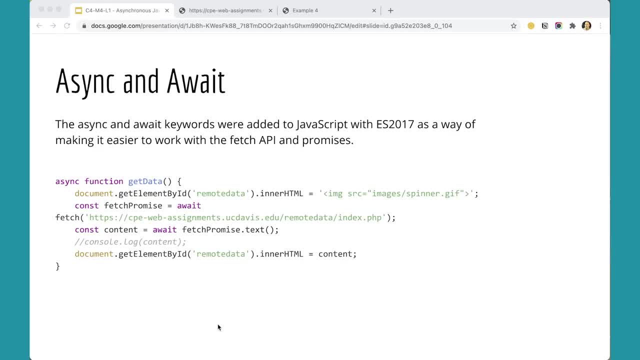 Plus, there's tons of articles about this stuff around the web, because everybody's trying to wrap their head around these new techniques And, ultimately, the really difficult thing about async and await is that it's easy to forget that you're working with asynchronous methods. 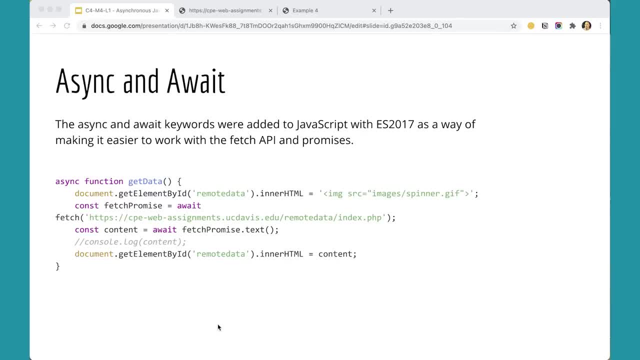 and to try to work with them in a synchronous way, the way we normally do, where things just happen one after another and to forget to put in await or forget to put async up here. It's really easy to forget to do that because it looks like normal procedural JavaScript, but it's not. 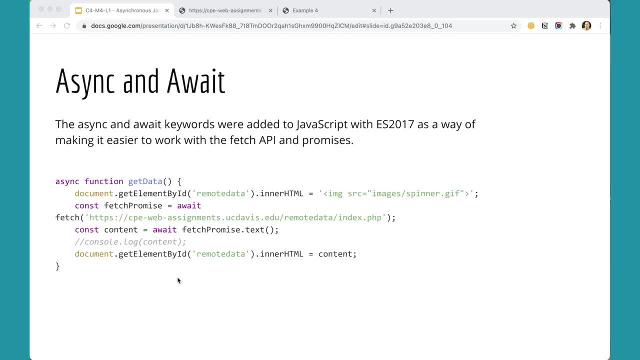 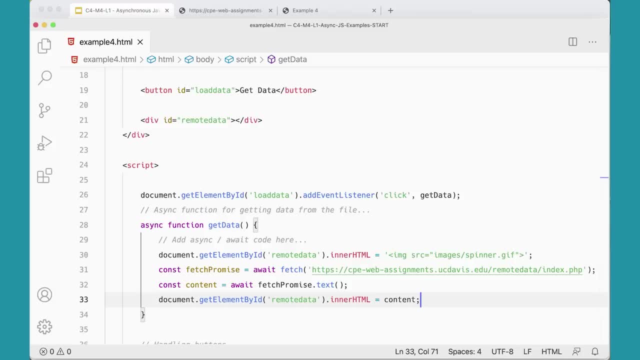 It's asynchronous JavaScript And that's really the hardest part You know when you look at this thing. it's not that complicated. Come back to our file. here We go and we put our spinner on the page, We go and fetch our remote URL. 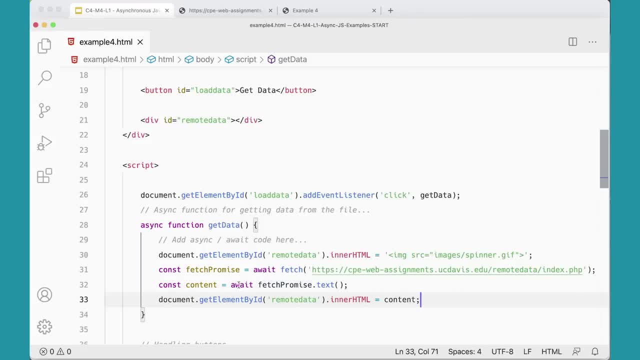 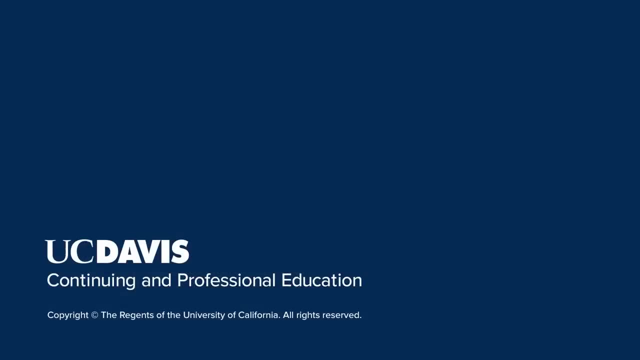 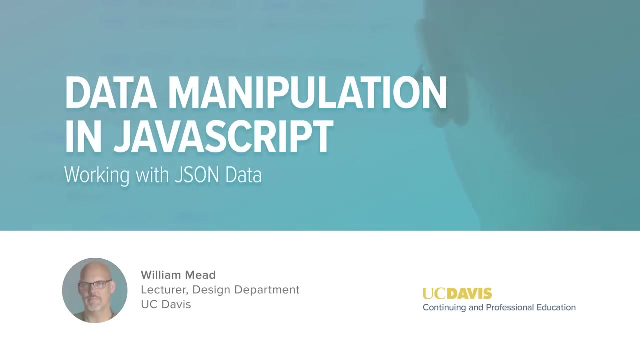 And we take that fetch promise text. We're waiting for it to come in. When it comes in, we're putting in content. When we get that content, we're putting it on the page. Pretty straightforward, Working with JSON data. In the first four examples: 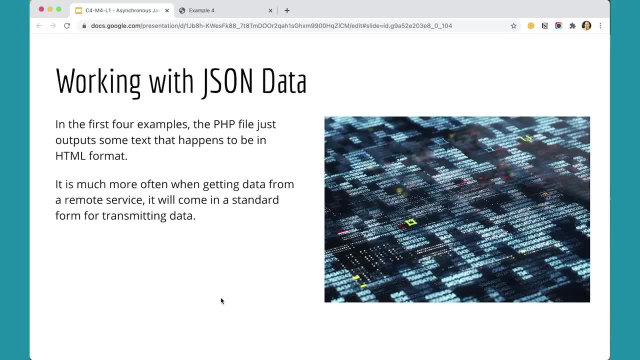 the PHP file just outputs some text that happens to be in the HTML format, So you can grab that HTML and just stick it on the page. No big deal. It's much more often that when you're getting data from a server, from a remote service. 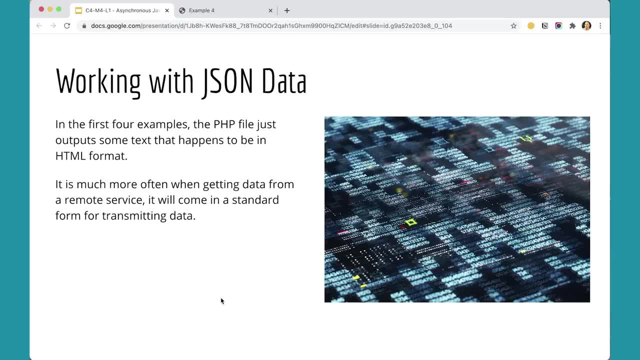 it will come in a standard form for transmitting data. The two most common formats for structured data are XML and JSON. XML is older. It has the advantage of including descriptive markup, but it's also heavier. JSON has become very popular and it looks very similar to the object syntax you're already familiar with. 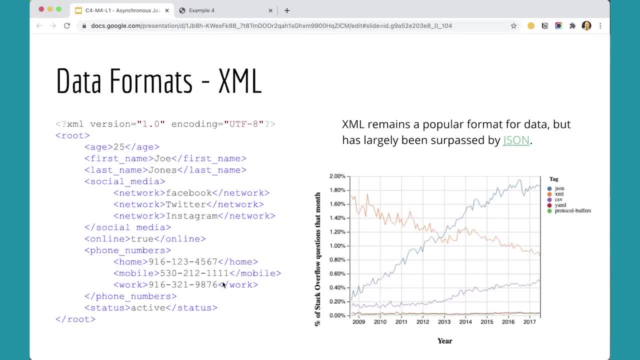 We've seen these images in a previous lesson, but it's important to include them here as well. This is what XML looks like, And you can tell by looking at it that it looks like HTML, And in fact, HTML is a subset of XML. 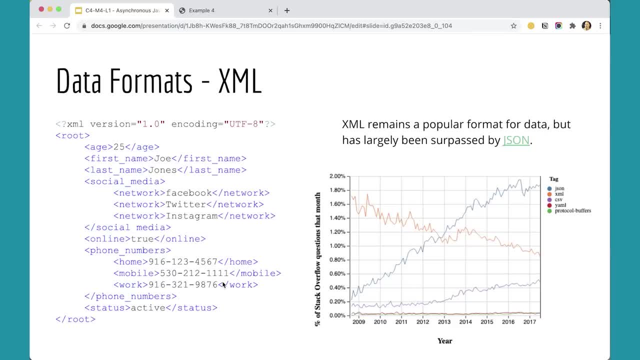 But in XML you can create any tag you want. You're not stuck with a specific set of tags like you are in HTML. You can use whatever tag you want, as long as it opens and closes, But- And it has that advantage of really creating structure for your data- 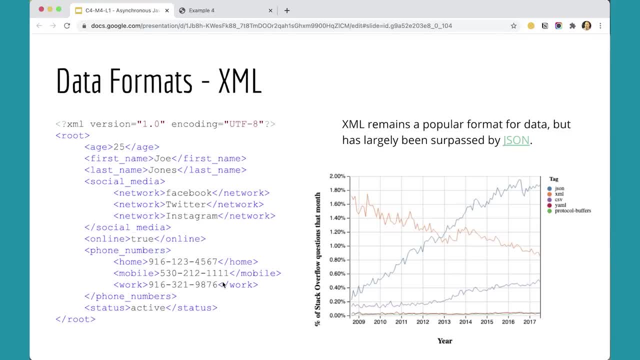 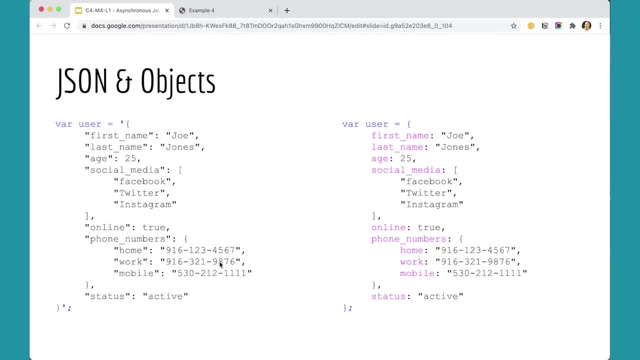 that you can see, But there's a lot of extra characters in there. If we look at the same thing in JSON, it's much simpler. So on the left we have JSON JavaScript Object Notation And on the right we have a JavaScript object. 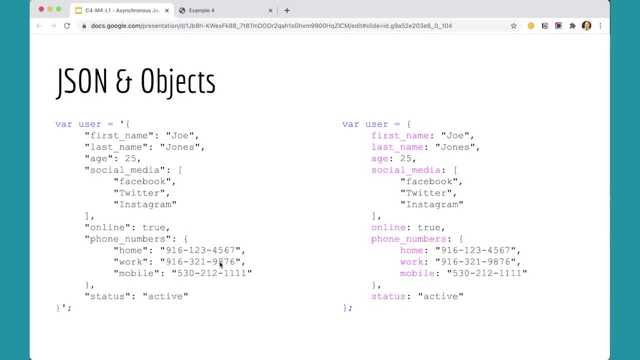 the exact same data in the JavaScript object- And again, we already looked at this when we looked at the lesson on objects- But here we can see that the data is much simpler, There's a lot fewer characters involved, But it also doesn't have quite the descriptive layer to it. 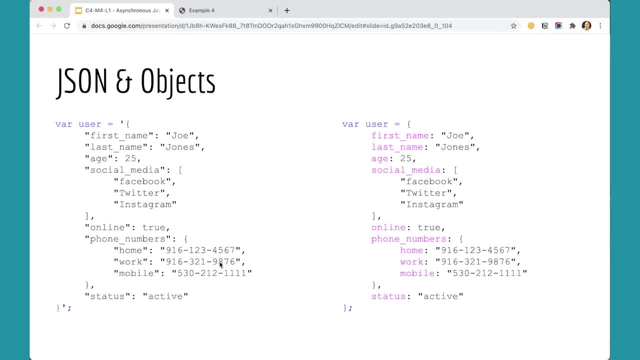 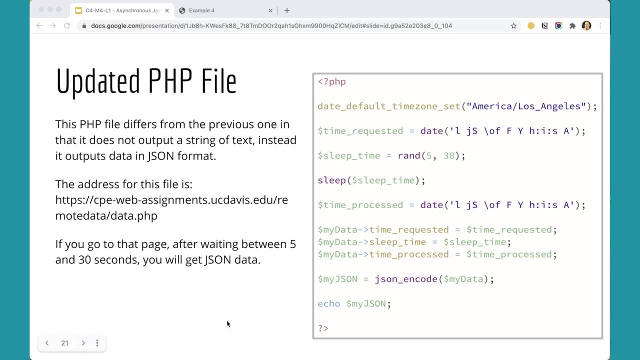 that XML has, But this has become very popular. I have an update to the PHP file that we've been using. The previous file doesn't outlive or output anything other than just some HTML, But this one instead outputs data in a JSON format. 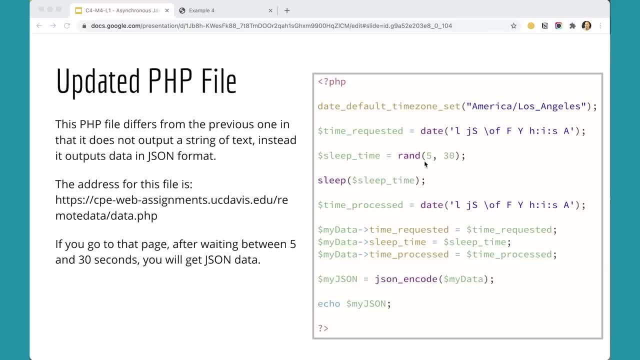 And you can see over here that this part's the same, This part's the same. All of this is the same We've got. The only thing that's different here is I've got an object that I'm sort of building up here. 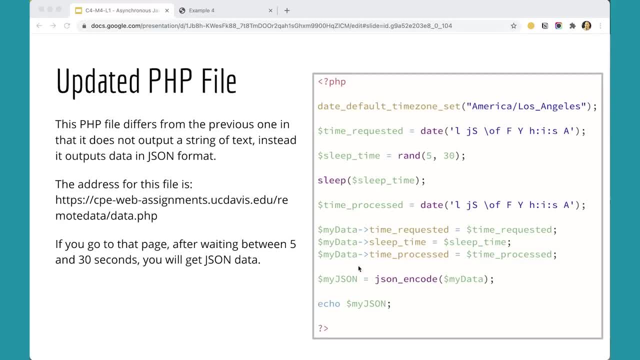 called MyData, which has these elements in it, And then I'm taking, I'm making a variable called MyJSON And JSON And I'm running this JSON encode on MyData, which will encode this and then echo out. print out my JSON. 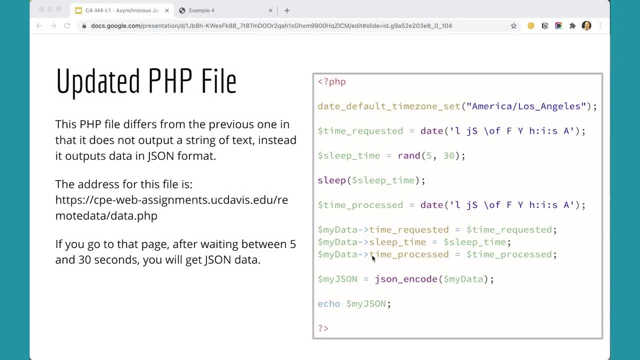 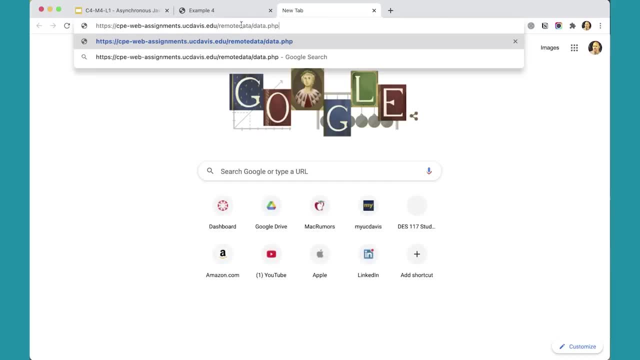 So this file simply outputs JSON data. Let's try it and see what happens. So if I go to a new tab here, I can paste in the URL for this. It's the same URL as before, except indexphp. It's dataphp. 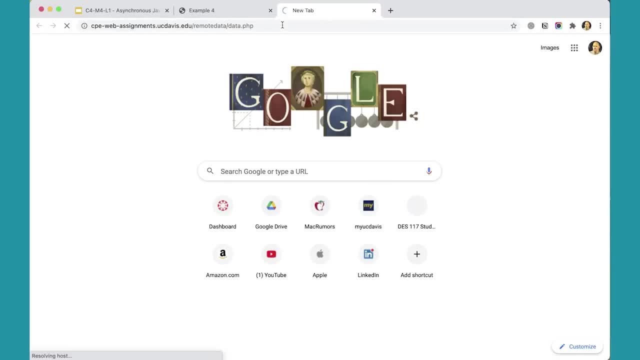 And I'm going to press Enter here And this is going to take between 5 and 30 seconds to process, While we're waiting for JSON to come through and get displayed on the page. But in the end, after however long it takes for it to do that, 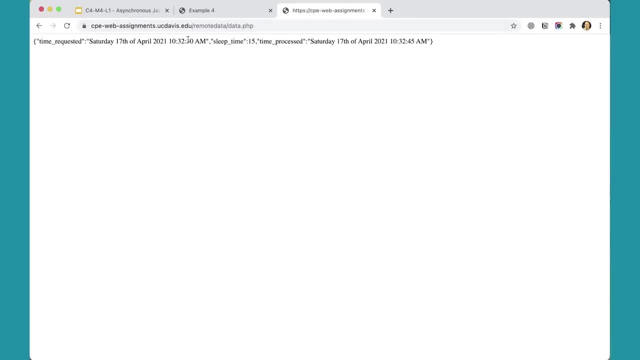 what we get is a string of JSON data. It's the exact same data that we got before in HTML, except now it's in JSON format And we can take that and parse that in our JavaScript. So let's take a look at example 5,. 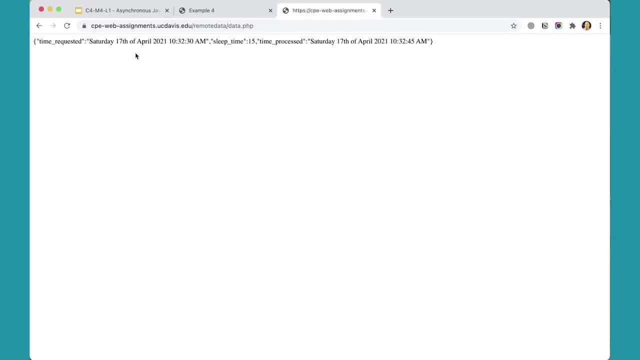 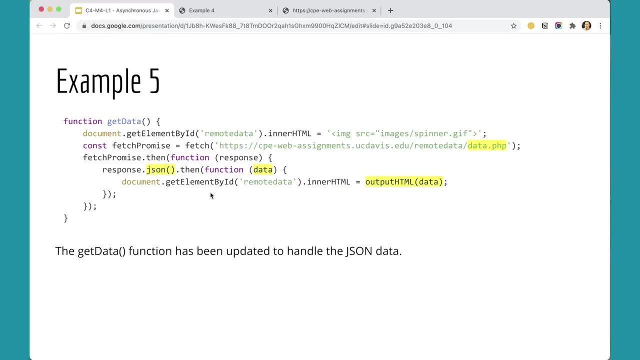 where we get to actually work with the JSON data. here In example 5, our function is going to change just a little bit. It's going to be very similar to 4, except it's going to change just a little bit here. 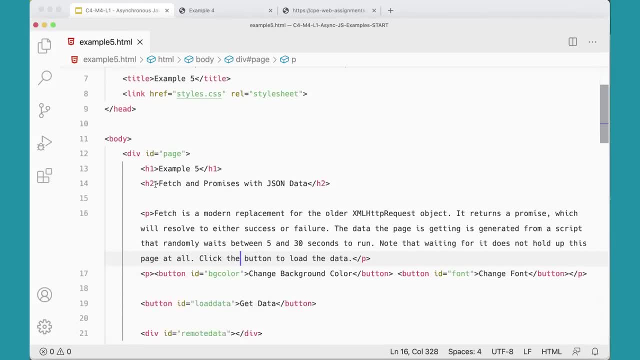 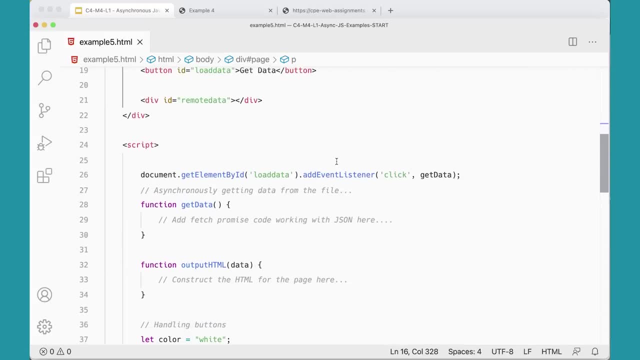 You can see that our example 5 HTML file looks very similar to what we had before. I still have my button, I still have my int and div, And down here I'm adding a click handler to my load data button that runs the get data method here. 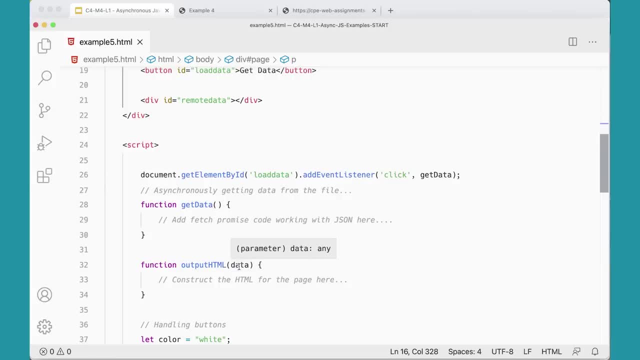 Now down here I've got an extra function that's going to pass in a parameter here that's going to actually construct the HTML for the page, Because before we were actually getting HTML from the server, Now we're getting just data from the server. 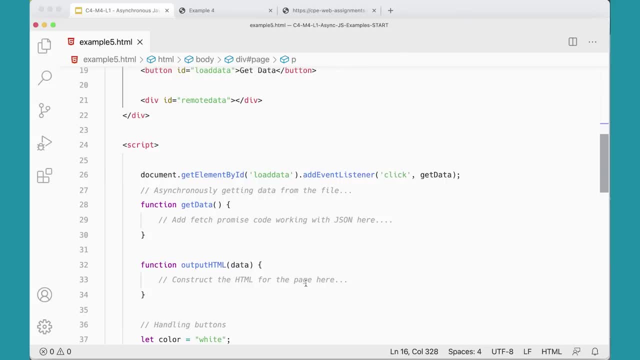 and we need to construct the HTML ourselves from that data. So we've got all this together. So the first couple of steps of this are the same as what we've done before. We're still going to put our spinner on the page, and then we're still going to have a variable for fetch promise. 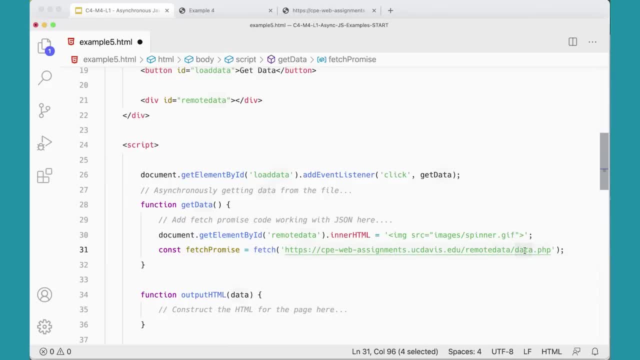 that's going to go get the data. The one thing that's different here is that instead of indexphp, we're now going to dataphp, which is our page. that's going to generate just some data instead of just HTML. So we've got those two pieces. 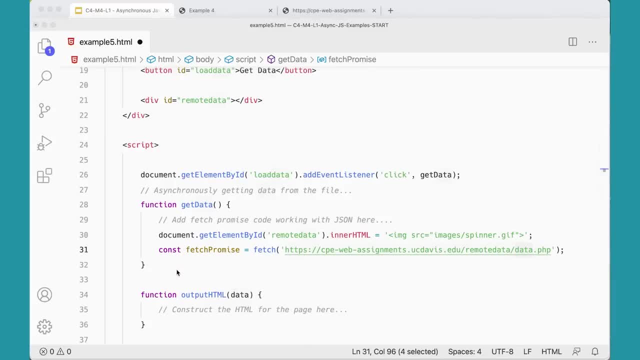 For this example, we're not using async and await. We're going to use the then method to get the promises and handle them as they resolve, as we did not in example four, but like we did in example three. So you can see how we're doing the same thing that we did in example three. 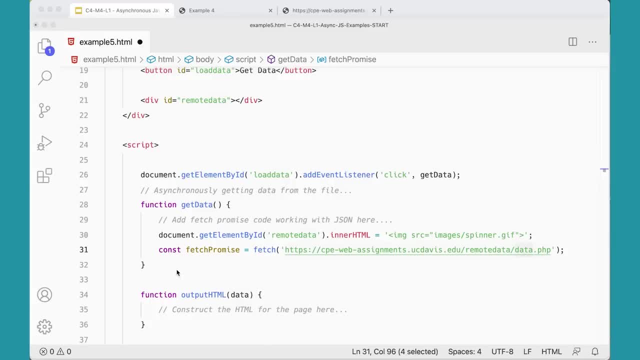 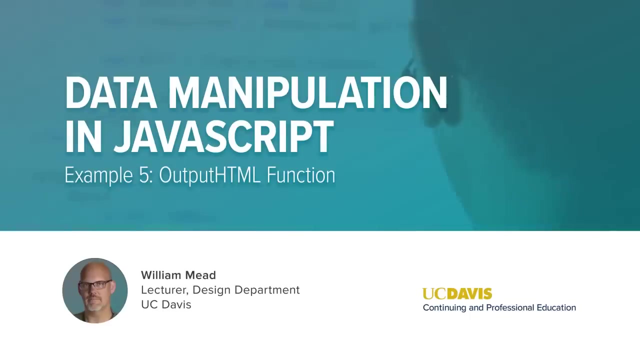 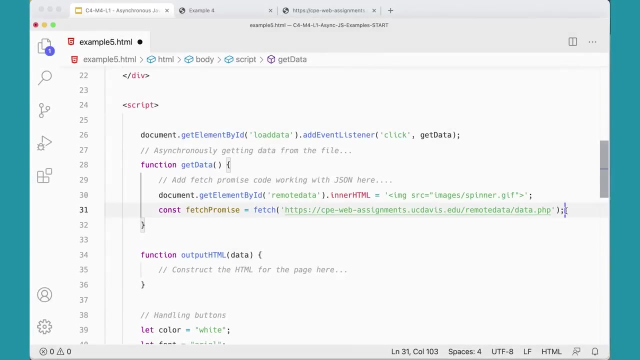 with fetch and the then method to process this data. But we'll pick that up in the next video So you can continue on with creating, working out this function here. In the previous video we started building out our function that's going to get our data, our JSON data, and work with it. 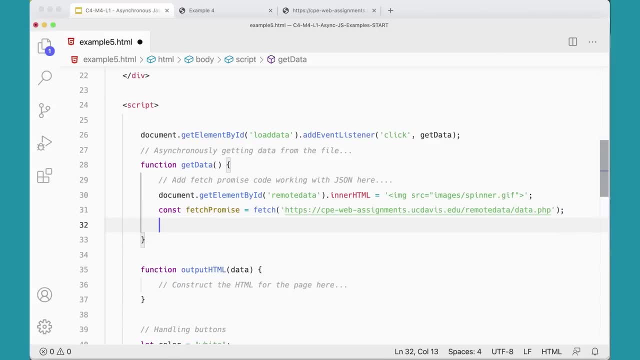 So, as before, as we did in example three, I'm going to take this fetch promise and I'm going to chain a then method to it to see what's going on And, as before, I'm going to pass in an anonymous function here. 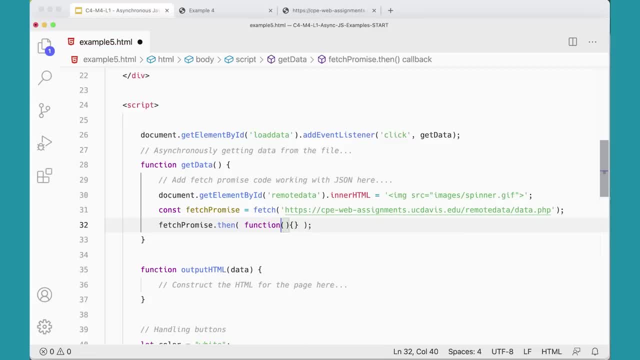 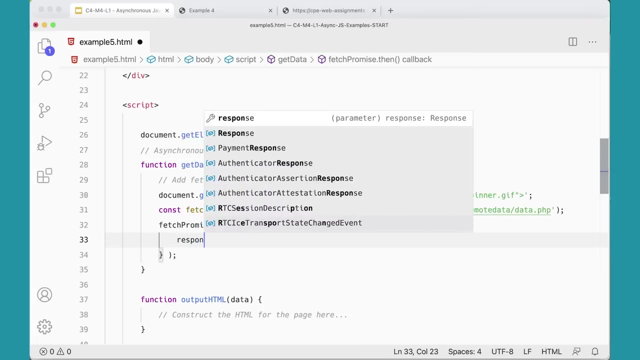 that's going to run And in that function I'm going to pass in the response object, because that response object is going to contain the response for what happens when this thing comes through. When the response comes back, the response is going to come back as JSON. 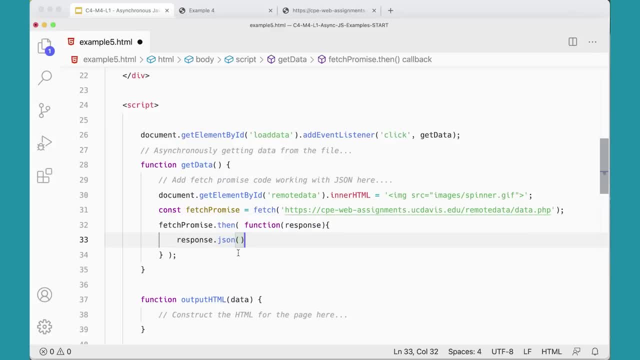 So instead of text, we're getting JSON back from this response. Once I've got that response back, I'm going to chain another then method on this here, on this JSON response, and again pass in an anonymous function That's going to get passed in here. 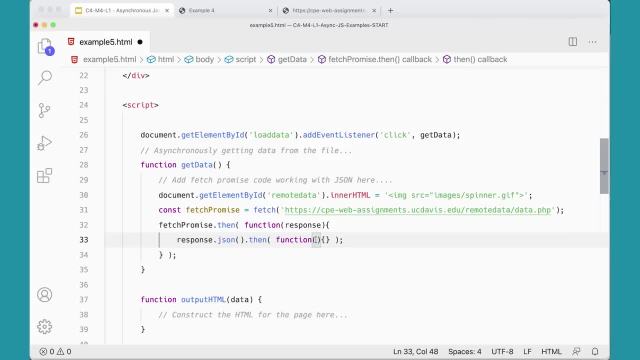 That function is going to get passed into it some data that came back from this JSON data here, And then we're going to go ahead and just take that inner HTML and run this output data. So output HTML data. we need to build out this function down here. 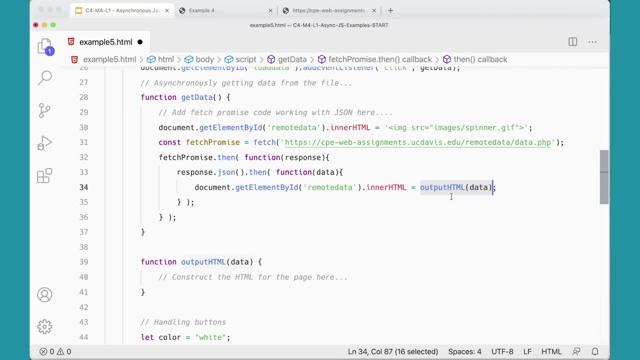 because data is just JSON, It's just data. So we don't want to stick just data on it. We don't want JSON showing up on the page. We want to actually take that data and put it in some HTML elements and display the HTML elements on the page. 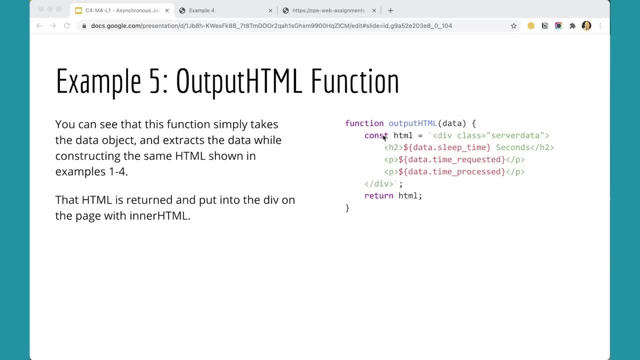 How do we do that? Well, this data is just data, So I can actually construct some HTML. So I have just a variable here called HTML And in it I'm using my tick marks. Don't forget the tick marks And they. 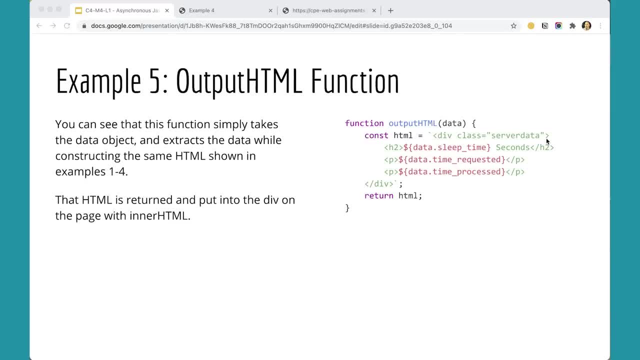 And I'm just setting up a div with class set to server data. A div closes down here at the end And then I can access the elements in this data: Datasleeptime, datatimerequested and datatimeprocessed. 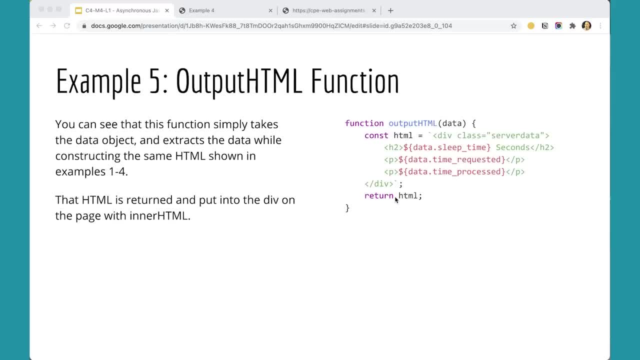 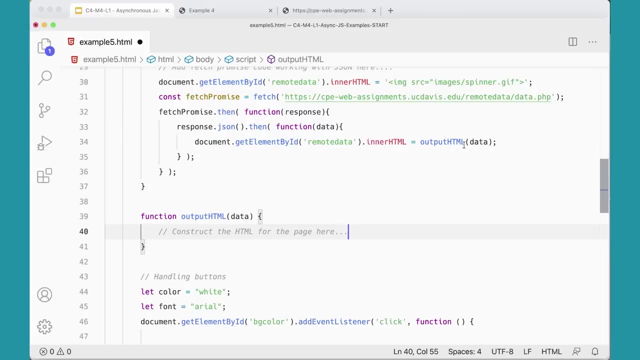 And I can just put them inside of elements, So we can go ahead and create the same HTML that we had in examples one through four, And then it just returns that HTML And we're taking that returned HTML and just putting it on the page here. 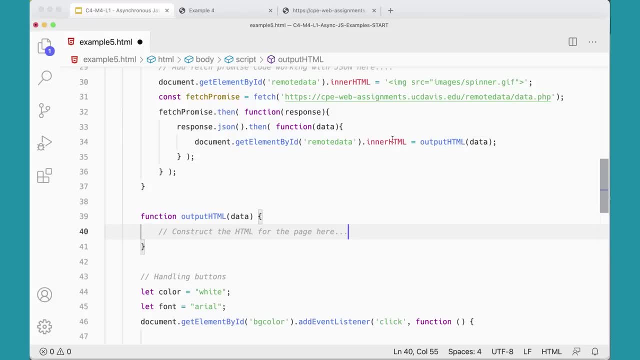 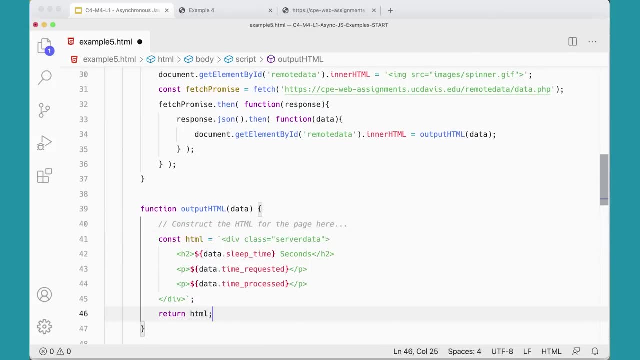 So this thing becomes the HTML And it gets put into the inner HTML. So down here I'm just going to add this And I'm just going to paste it in. You're going to have to type it, But I figure it's not really worth watching me type it. 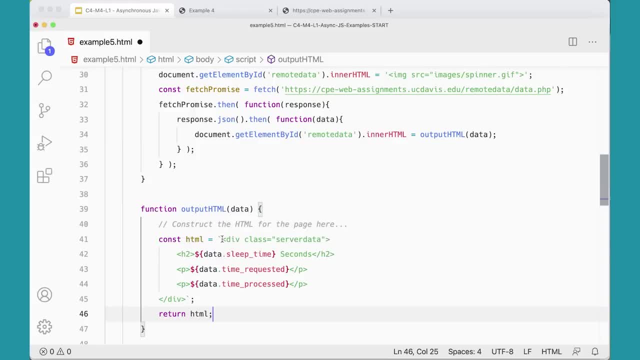 because it's just a variable that's holding a string And it's a string template here in that it's got the tick marks, So you got to make sure you get your HTML And type this all correctly. But these are just variables. 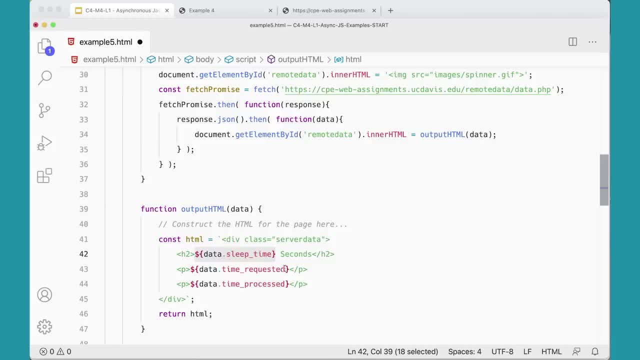 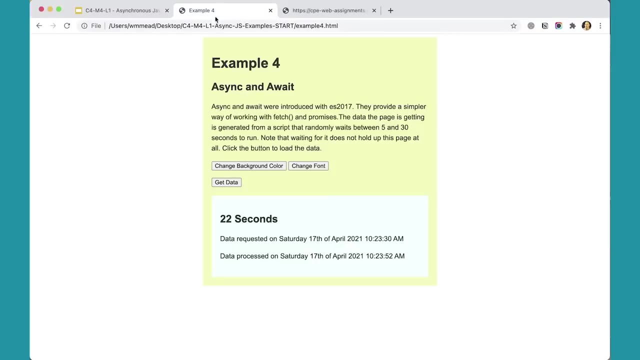 Datasleeptime, datatimerequested and datatimeprocessed is the data that we're getting from our form. OK, great, So let's give this a try real quick. This should actually work. If I come back to my browser up here, I'm looking at example four. 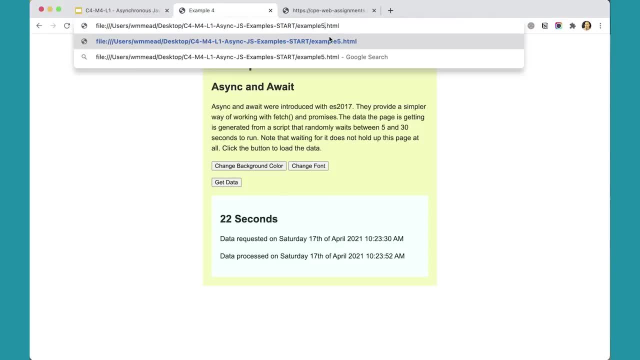 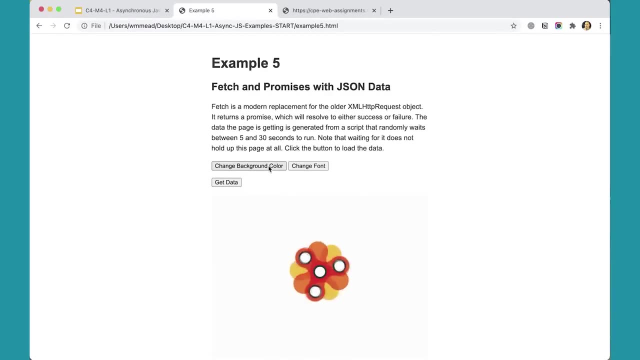 I'm going to change that to example five: Hit HTML. Here I am on example five. If I click Get Data, I'm getting my spinner. It's doing its spinny thing while it's waiting for the data. I can do things like change the font and the background color. 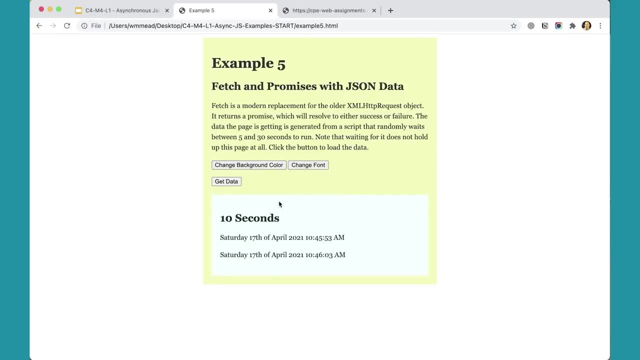 so it's not blocking anything- Same as before, And this time it took 10 seconds to complete, So that's really pretty awesome. So you can use the fetch and the promises with JSON data, which is really just generating a string of data. 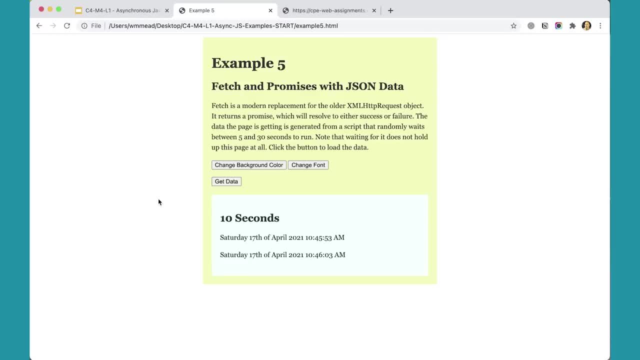 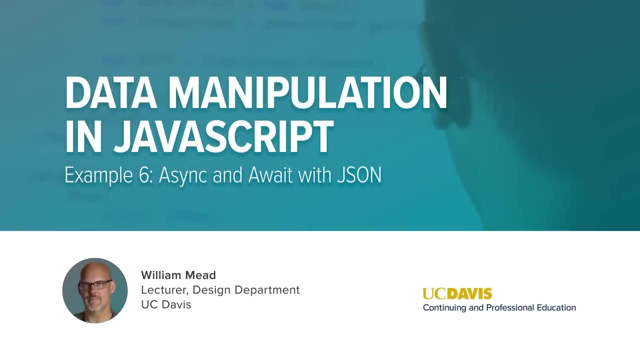 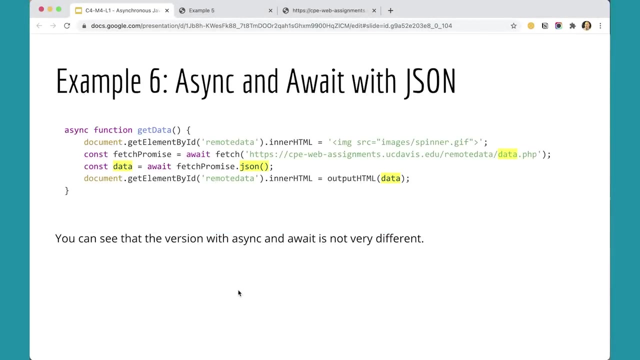 And most of the time, if you're working with an external service, they're going to be giving back data in some sort of standard format, And JSON is the most popular format out there these days: Insert. As you probably guessed, you can use async and await with JSON as well. 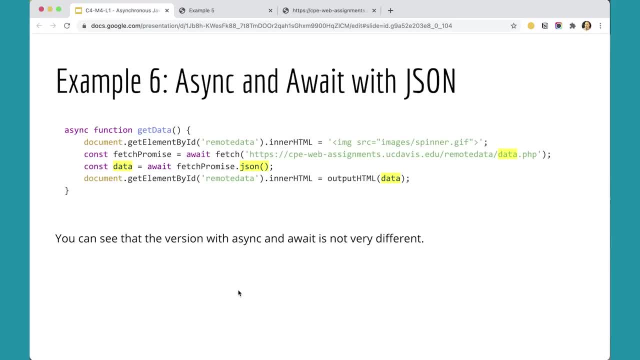 There wouldn't be much use without it, because most of our data is coming in a JSON format anyway. So we need to be able to use async and await, And you can see here that this updated version of the Get Data function is still only four lines long. 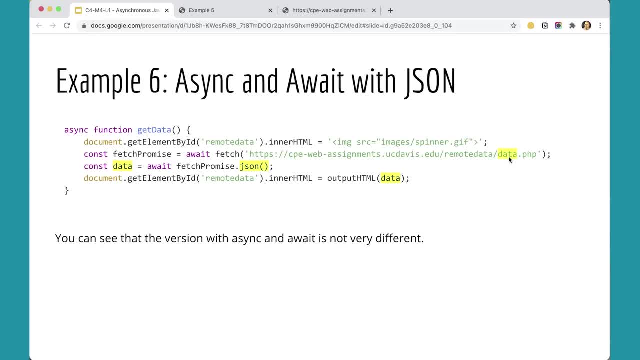 And the only things that have really changed is that this is now data instead of indexphp. Down here I've got a const data that's just getting the fetch promise here and getting JSON And we're using await. We're using await there. 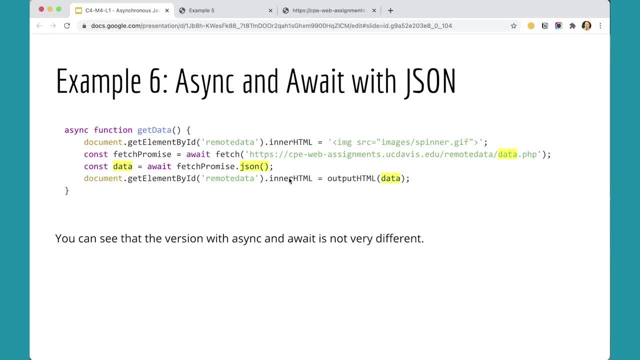 That's the same as before. And then when that comes back, we're just taking that data and running it into the output HTML function here We're passing in data here now, But this function has not changed at all. It's really the exact same thing as it was before. 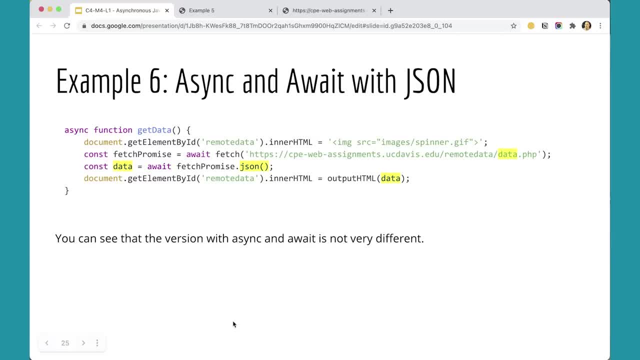 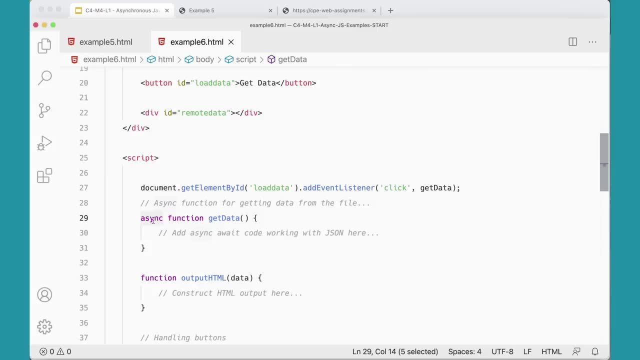 So that's pretty cool. Let's go ahead and get this in place, because we want to test it and make sure it all works. We have our async function with the async keyword in front of it, And then we're going to paste in. 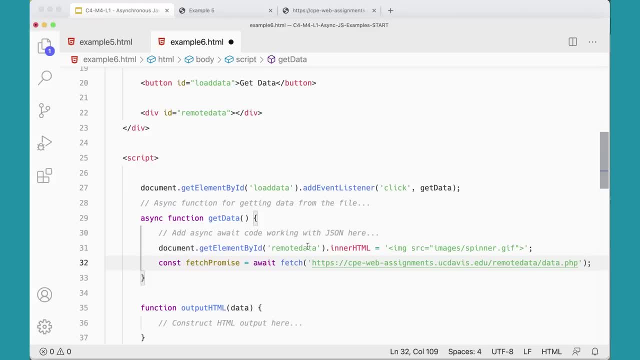 I'm pasting it in. You're going to have to type it. Document get element by the remote data in your HTML. You can copy this from one of the other files because it hasn't changed. It's the exact same thing. This hasn't changed. 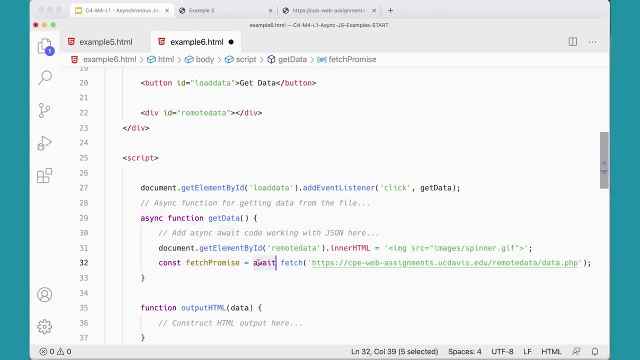 The only thing that's different here is that now I have await in front of it, But it's going and getting the dataphp file that we need. Then, as before, we've got a variable called data. I've changed the name to data now instead of text. 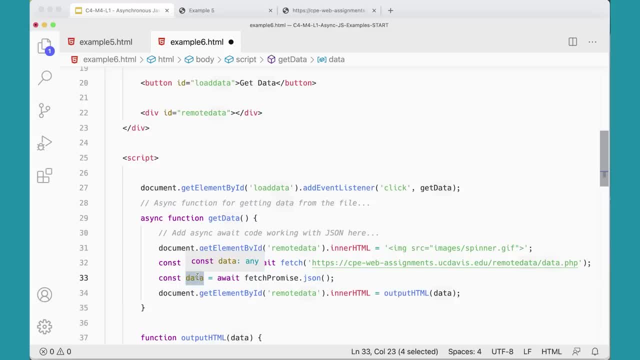 because it's data, But it could be anything. You can call this variable whatever you want, But I'm awaiting that fetch promise, the JSON to come back from this fetch promise. here I'm awaiting, I'm waiting for it to come back. 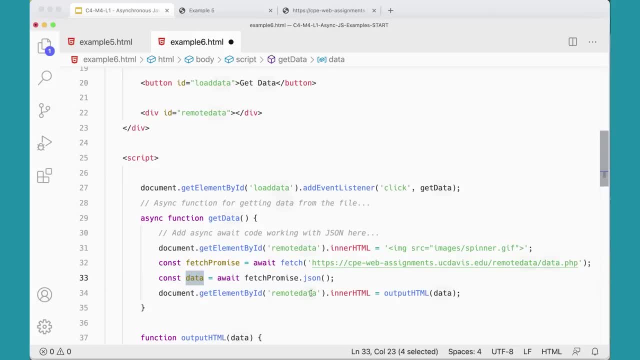 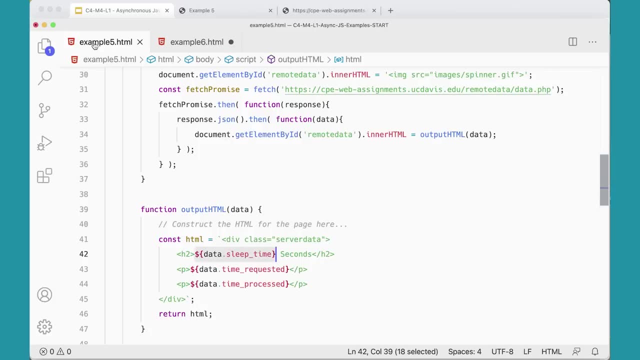 When it does this will have something in it, And then I can just put it on the page: output data. Down here I've got my output data function, But this function is exactly the same as before. I can go to example five here. 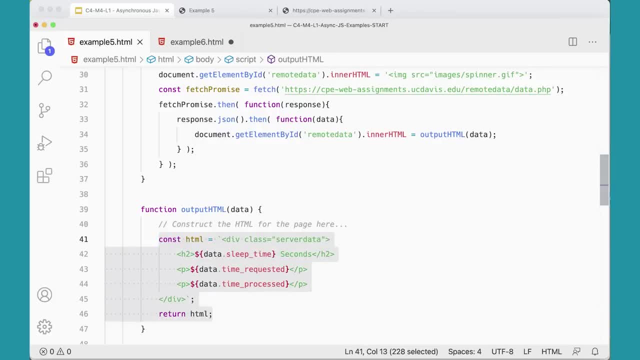 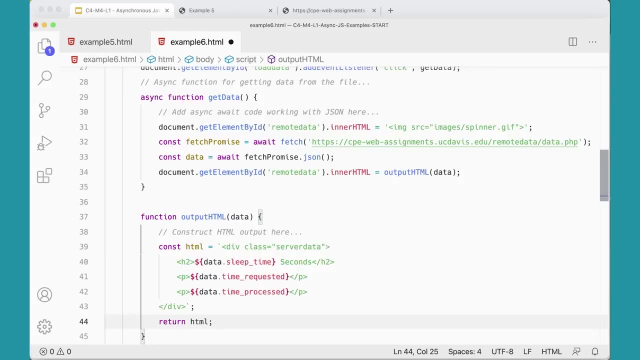 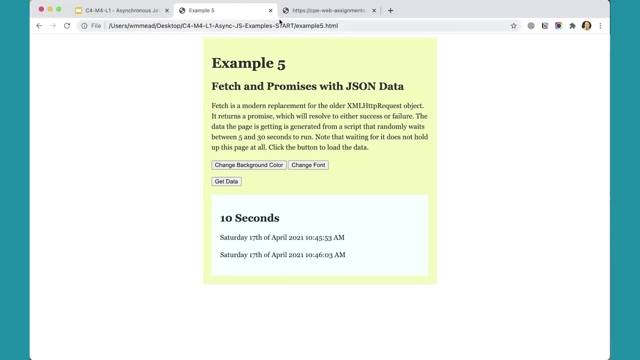 and just copy all of this from here and paste it in there. It's not any different than it was before at all, So I can just put that in And that should just work. So if I come back to my web browser here and pull up example six instead, 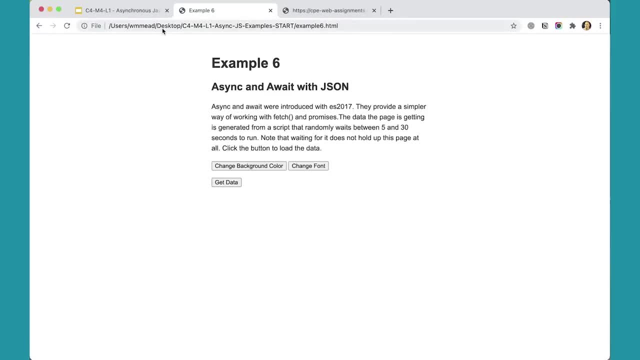 And notice, I'm just using these files from my desktop. They're just here on my desktop. I don't have to do anything fancy, I don't need to be running PHP or anything like that, because the PHP is all happening on the server. 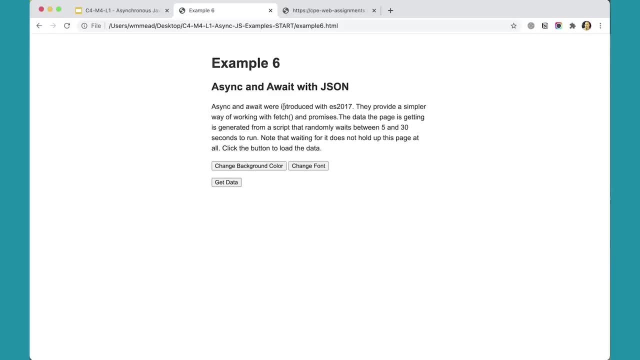 If you wanted to run the PHP file that goes with this, you would need a server to run it on, But you might as well just run it from our server here, the cp-webassignmentscom, So you can see what it does. All right. 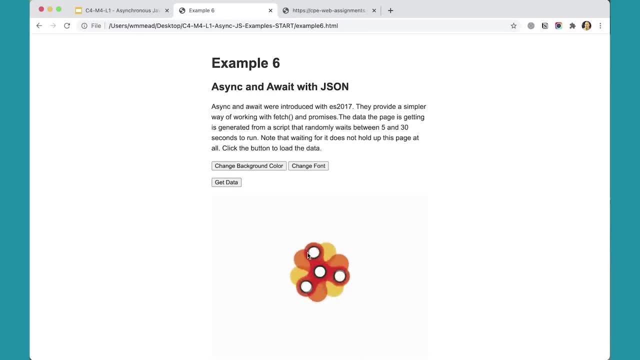 So let's see if it works, Let's see if I did that right. I'm getting my spinner And it's running forever long that it needs to run, And I can change the background color, I can change the font, so it's not blocking anything. 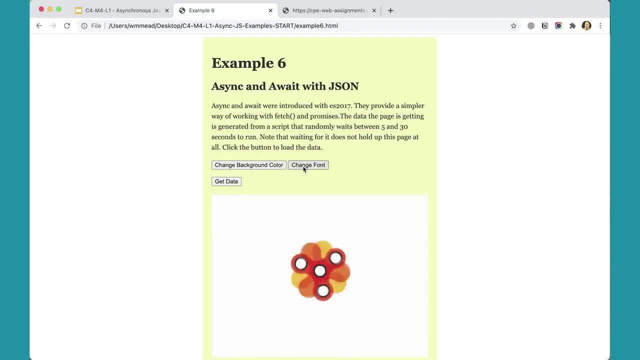 Sometimes you'll hear JavaScript is described as non-blocking, And this is what they're talking about: is that we can use asynchronous functions to go off and do something And JavaScript will just put in and put it aside and wait for it until it comes back. 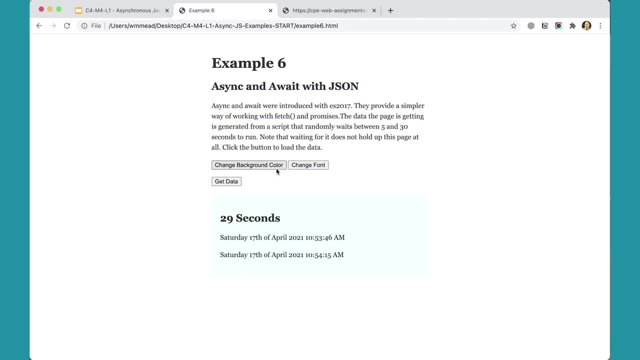 And meanwhile we can do other things, just like in our kitchen metaphor there. So we can do that, And it took 29 seconds- almost the total length of time available- for it to come back and finish and fill this thing out. 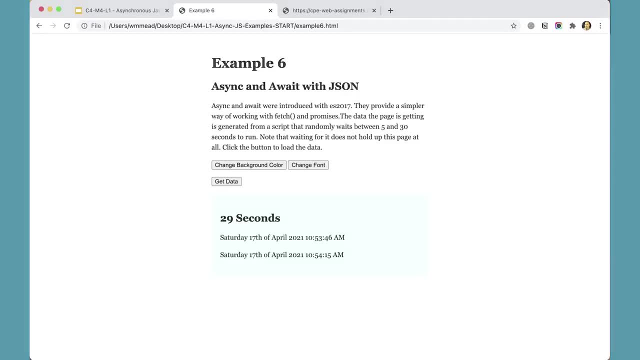 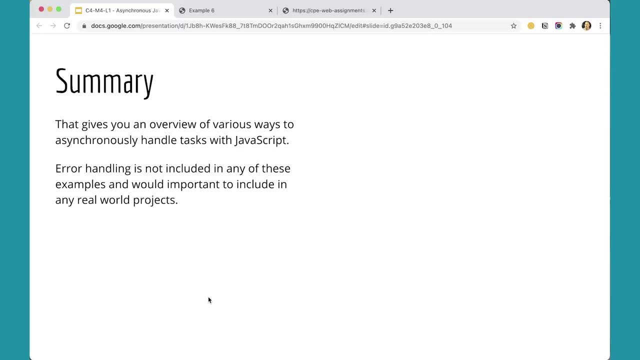 But it's working great And that's really cool. Summary That gives you an overview of the various ways to asynchronously handle tasks with JavaScript. It's important to note that error handling has not been included in any of these examples, And it would be important to include. 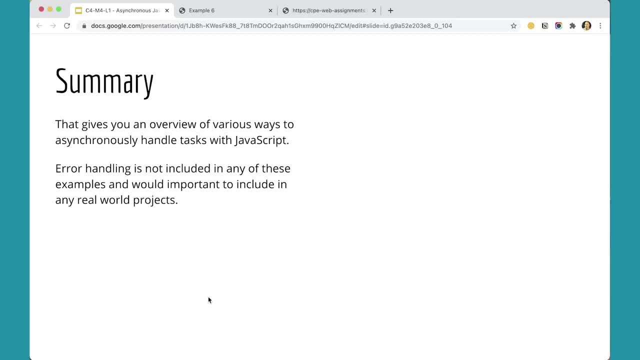 in any real-world projects, And we'll look at how to do that in a future assignment. Also returning to the cooking analogy, we're not doing much more here than watching the toaster toast bread. The asynchronous functions become a lot more interesting when they start to pile up. 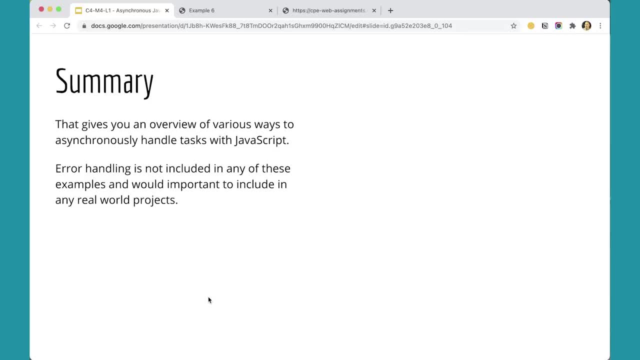 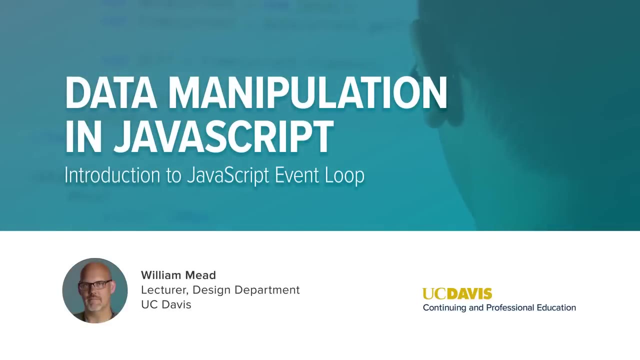 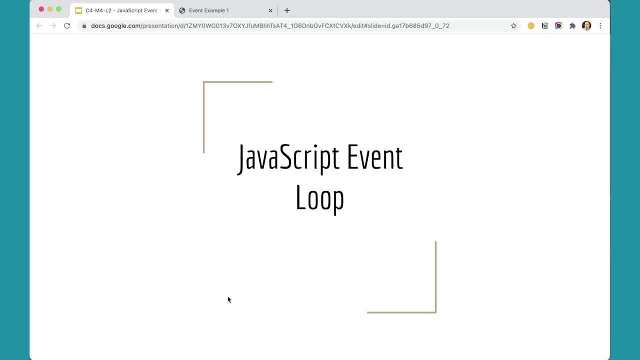 and your program is doing multiple things at once, like having many pans on the stove. Okay, great, I'll see you in the next lesson. JavaScript event loop. The concurrency model in the event loop in JavaScript is different from what you would see. 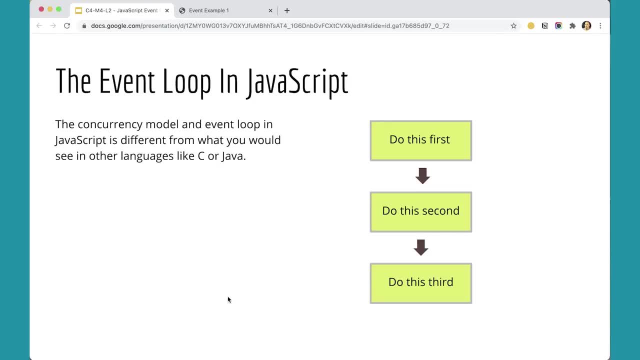 in other languages like C or Java. Now that you're working with some asynchronous functions, it's important to understand it just a little bit better. JavaScript is single-threaded and can only do one thing at a time. We've already talked about that in the previous lesson. 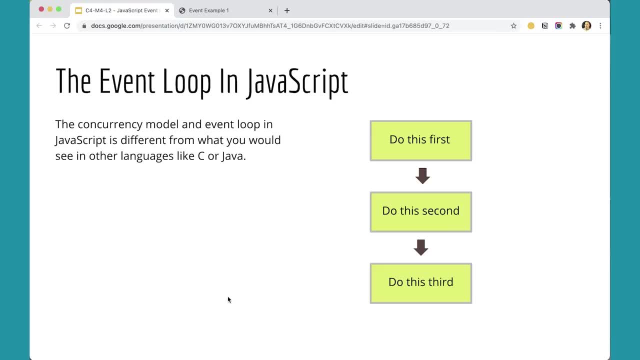 This provides certain advantages. As a function runs, it will complete its task and do whatever it does with application data until it's done, without interruption from another task or function. So it'll do this first, then it'll do that second, and then it'll do that third. 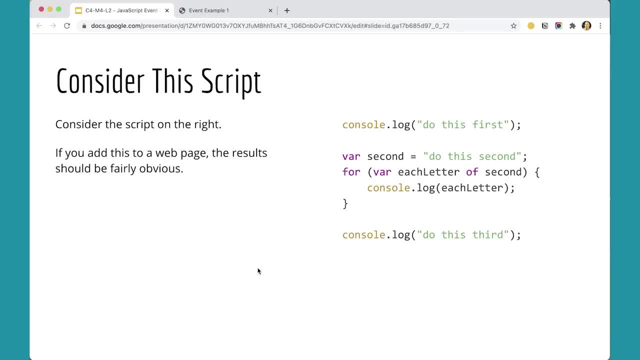 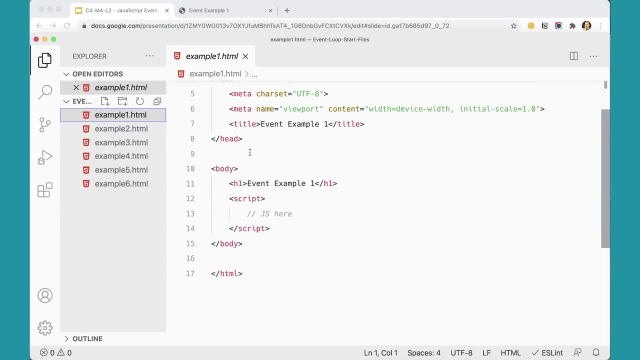 Let's consider this script on the right here. If you add this to a web page, the results should be fairly obvious, So let's go ahead and do that In my code editor over here. I have example one open here and I'm just going to add some JavaScript here. 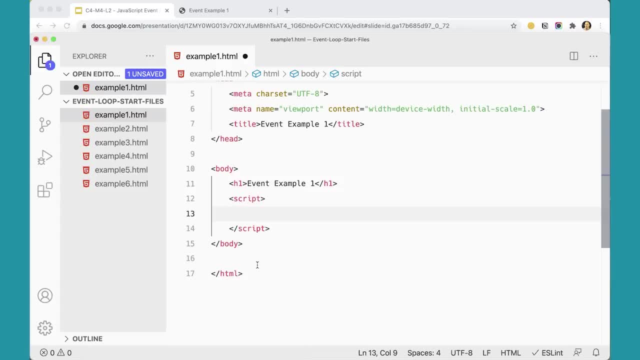 Don't really need that comment. I'll start by just console logging out: do this first. That's pretty straightforward. We know what that'll do. That'll send a message to the console that says: do this first. Then I'm going to make a variable called second. 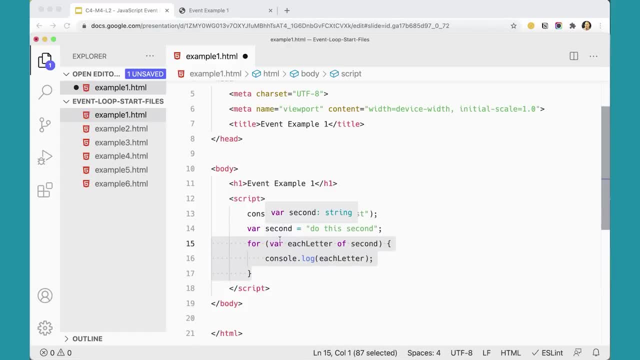 and it says: do this. second is in this variable. second, Then I'm going to use a for of loop, So for var. each letter of second console log, each letter. So what that should do is go through and loop through each letter of this variable. 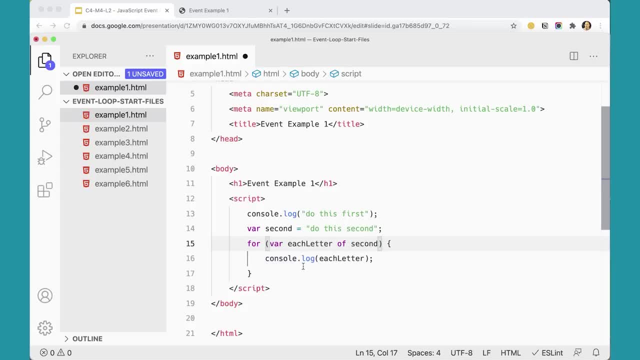 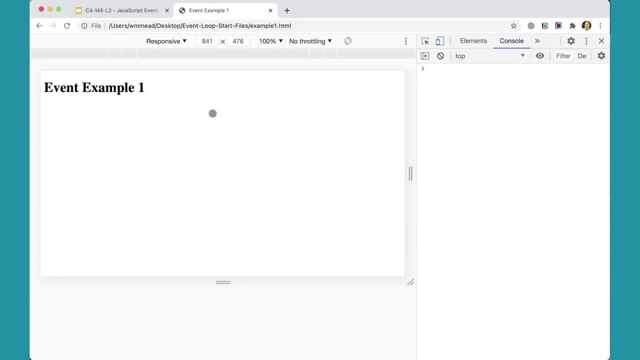 and console log it out one at a time. Great, pretty straightforward. Then I'm just going to console log, do this. third: So if I save this and then come over to my code over here, to my browser here, and refresh this page, 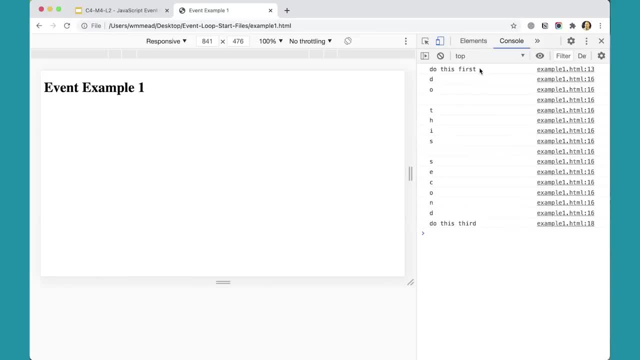 the results should not be that surprising. It did this first, and then it printed out each letter. It did that entire loop, completed the entire loop with all of that data in it, and then it did the third thing. It just does them one, two, three. 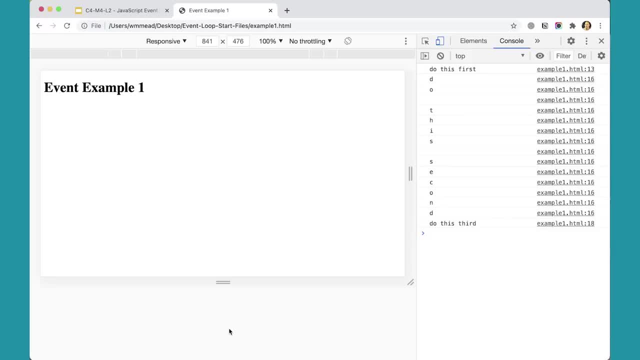 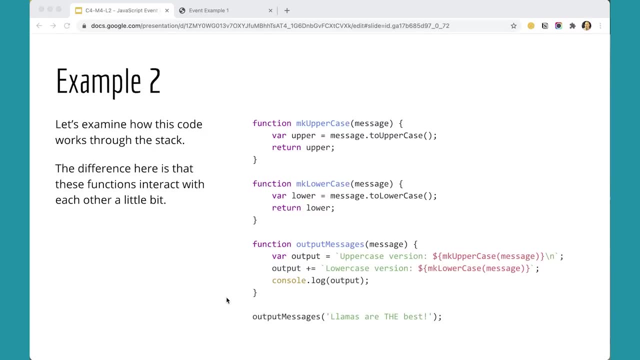 No big deal. That's the normal procedure that we're used to seeing in JavaScript. Let's take a look at example two and how this code works through the stack of things to get done that JavaScript has to do. The difference here is that the way these functions interact with each other a bit. 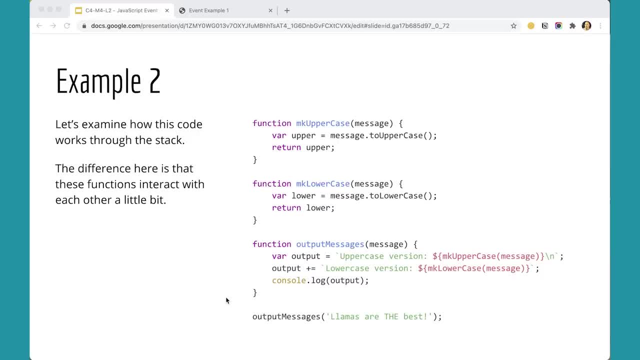 In the previous example, one thing did one thing and it went on to the next, and so on and so forth, and nothing really interacted with anything else. in terms of the functions, Here we start with a function that takes a message, makes it uppercase. 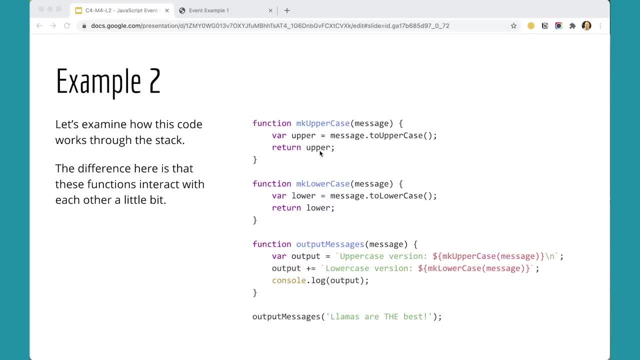 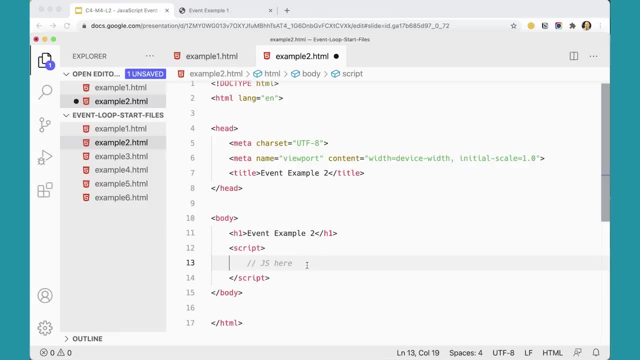 and then returns that variable upper. when it's done, Let's go ahead and add this over to example two here. Here I've got js here. I'm going to take that out and just add this function here. I'm pasting it in. 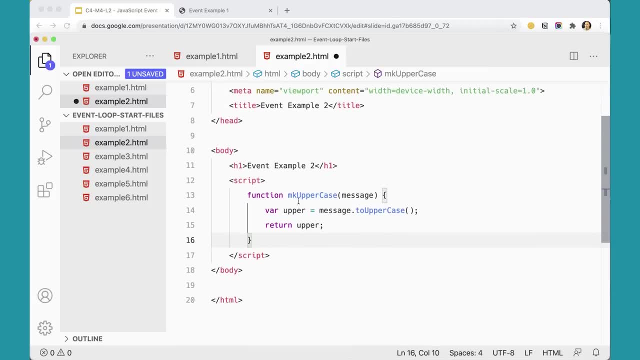 but you're going to have to type it in. That's make uppercase. That's a function that does that. When the script runs, it defines that function, so that's great. Then we've got the same thing for a function that makes messages lowercase. 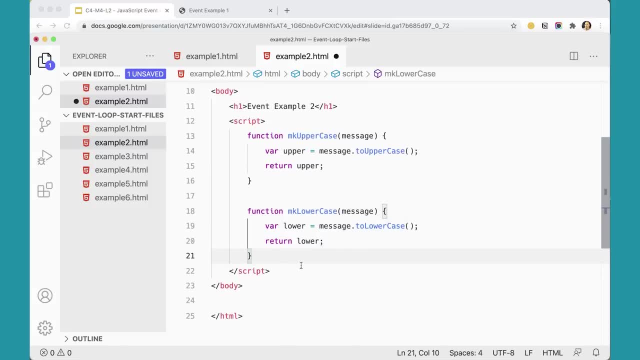 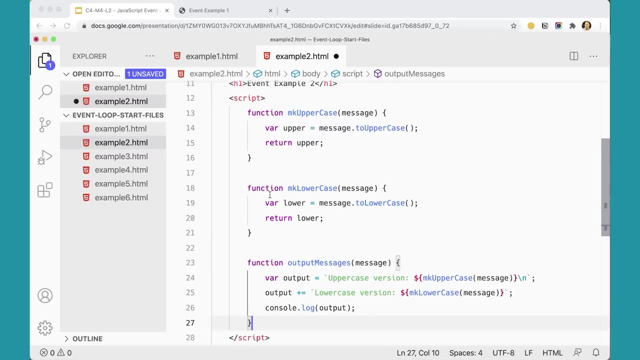 It does the same thing, but it makes messages lowercase. That's great, We've got that. Then we have a function- You're going to have to type it out: Output messages takes that same message and then we have a variable output. 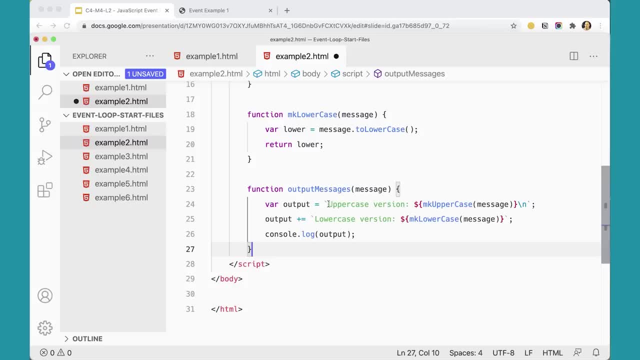 that's going to include a string template here where we've got the upper version, and then that's going to hold in it a variable that's really running the make uppercase version and then a line break. Then we're going to add to that output. 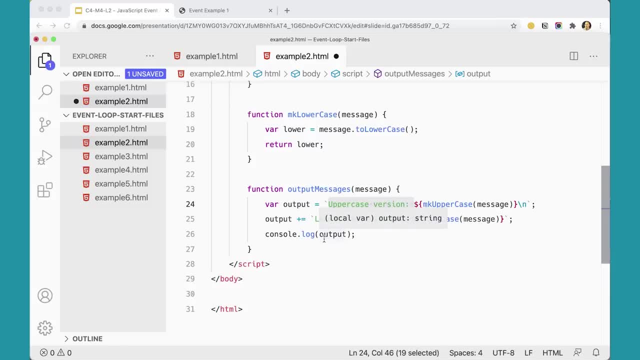 a lowercase version that's going to run that one, and then we're going to console log out the output. Finally, I actually run this third method here, this third function here, passing in a mixed case message that I'm going to pass in here. 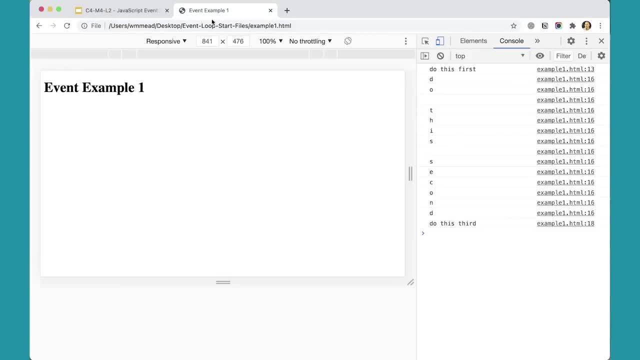 Let's see what that actually does when we run that over here. I'm going to come over here to example two. You can see I've got an uppercase version and then I've got a lowercase version, so it's actually functioning. It did all of that stuff. 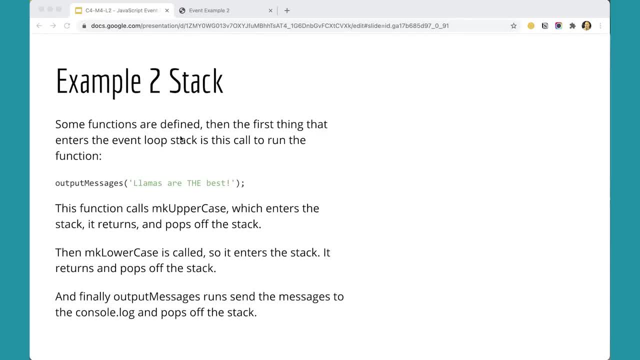 For this example, some functions are defined, Then the first thing that enters the event loop stack is the call to run the function output messages. That enters the event loop, Then the make lowercase is called, so it enters the stack, It returns and pops off the stack. 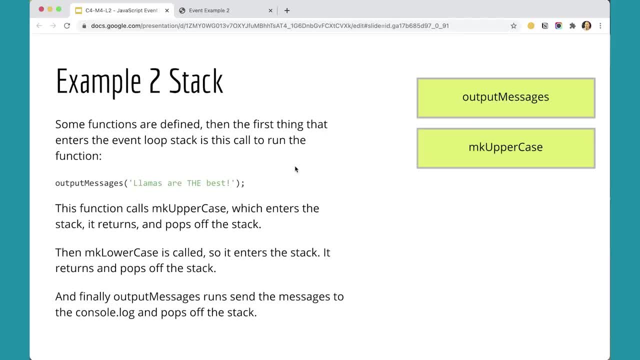 That comes in, it does its thing, and then, when it's done, it returns and off it goes. Finally, output messages. then the lowercase one comes in and it enters the stack. It does its thing and then it pops off the stack. 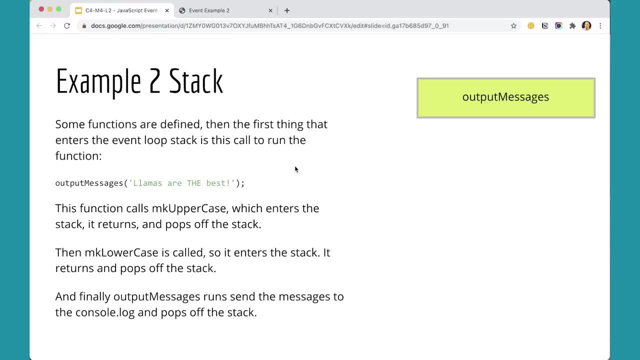 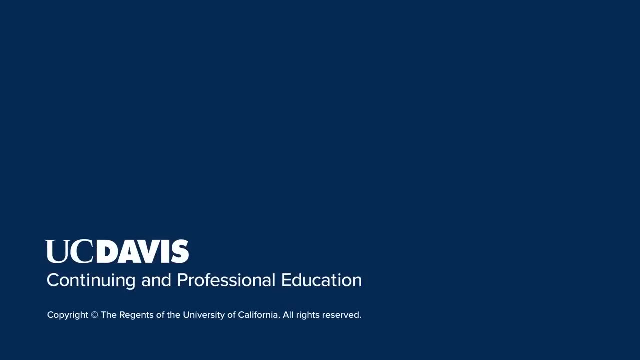 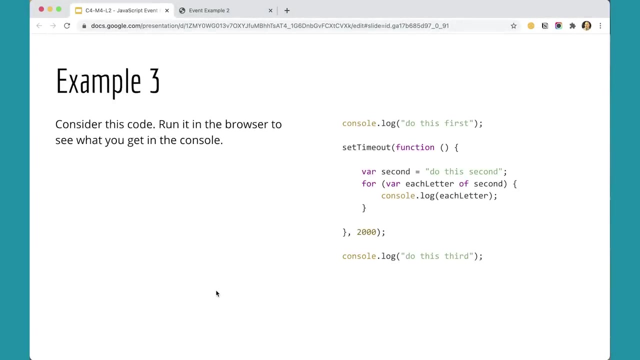 Finally, output message runs and sends the message to console log and pops off the stack. That's how that particular example runs from the event loop stack perspective. Example three: Let's consider this code and run it into the browser to see what we get in the console. 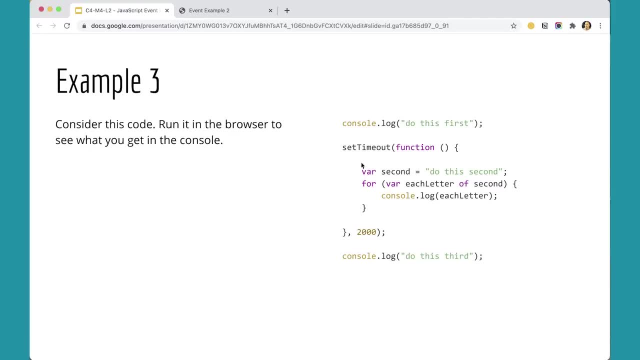 It's very similar to example one, except we're using setTimeout, which we've looked at in a previous lesson. Let's go and take a look at example three here. I'm going to go grab example three. Really, what I'm going to do. 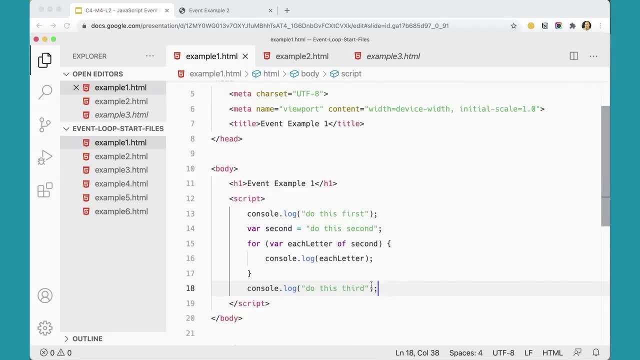 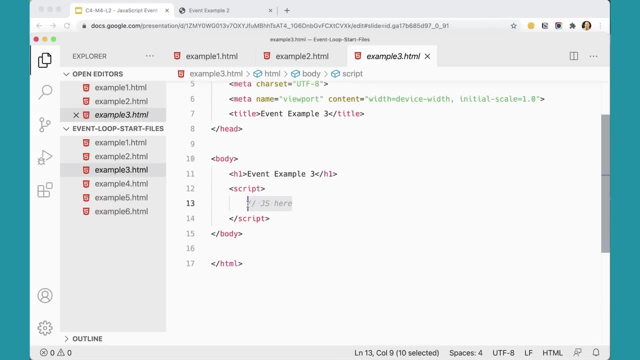 is. I'm going to just copy and paste from example one. I'm going to have to type all this all over again. I'm going to come down here. I'm going to add this in here Here. I'm going to put in: 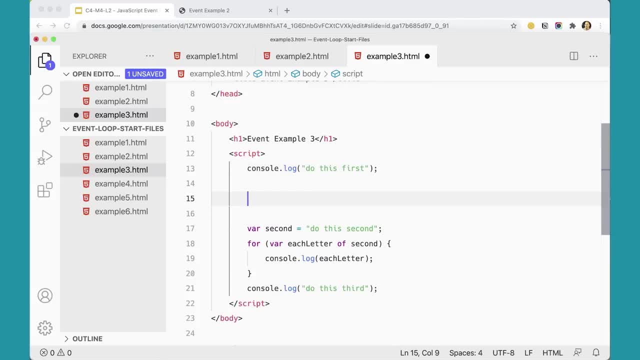 a call to setTimeout, I'm going to do setTimeout. setTimeout, we know, takes a function and then a period of time. In this case I'm using two seconds- And then, inside the curly braces, I'm going to stick just these pieces here. 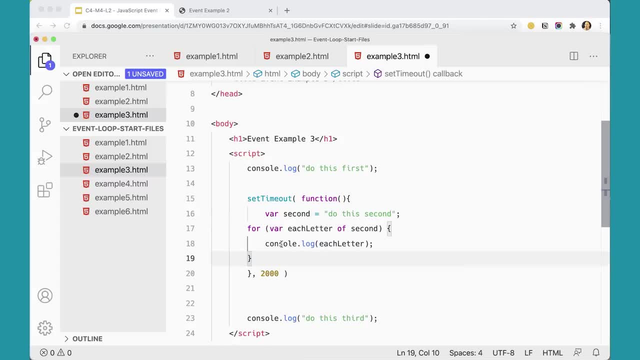 I'm going to do setTimeout And then, inside the curly braces, I'm going to do setTimeout, And then, inside the curly braces, I'm going to do setTimeout. So now the setTimeout is going to wait two seconds before it does this. 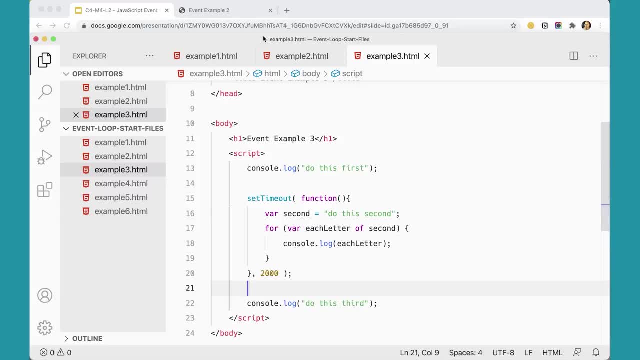 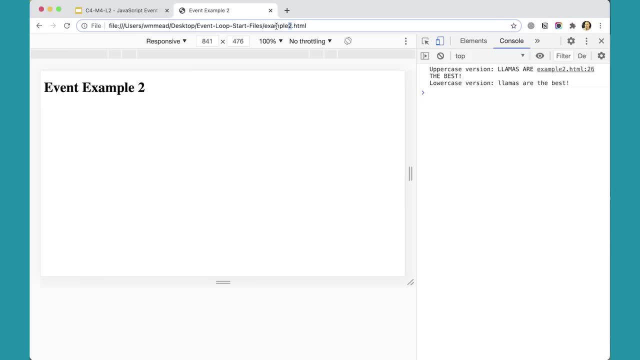 Let's take a look at this version in the browser and see what happens here. If I come over here and load up example three and load up example three, you'll see it did the first one first and then it did the third thing. 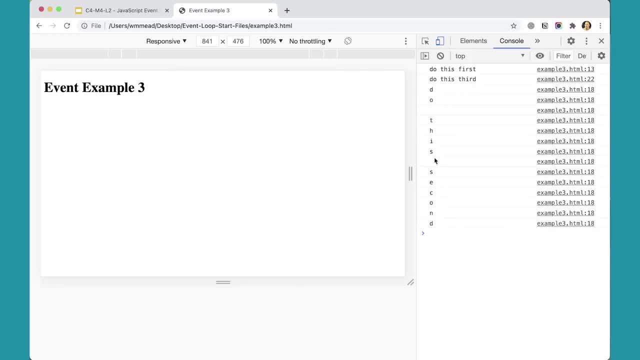 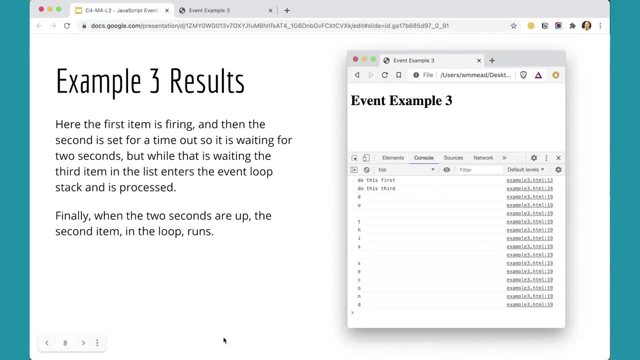 and then the loop that it said to do. second, it did last. So here the first item is firing, but then the second is set for a setTimeout. So it's waiting for two seconds. But while it's waiting for that to happen, 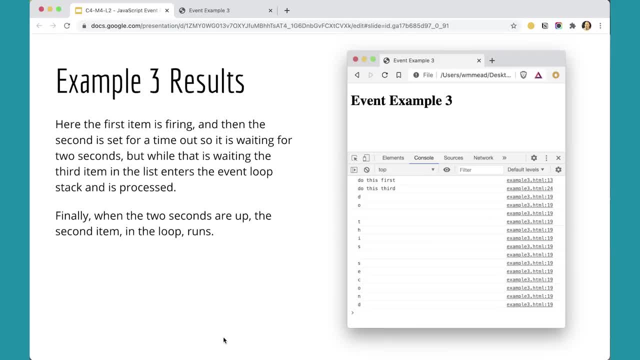 the third item enters the event loop in the stack and is processed. Finally, when the two seconds are up, the second item in the loop runs. So when JavaScript encounters setTimeout it kind of puts it aside, kind of like the toaster that we were watching while. 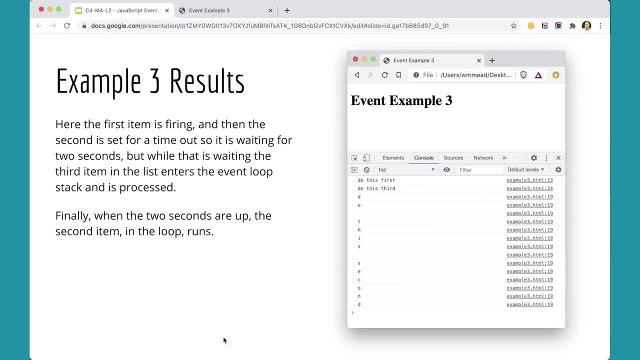 you know that we're not going to watch while it's toasting the bread. It's just when it finishes its time it's going to ding and say I'm ready, and then JavaScript will come back to it. But meanwhile 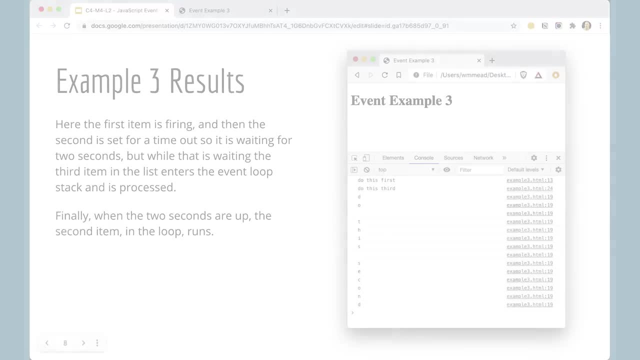 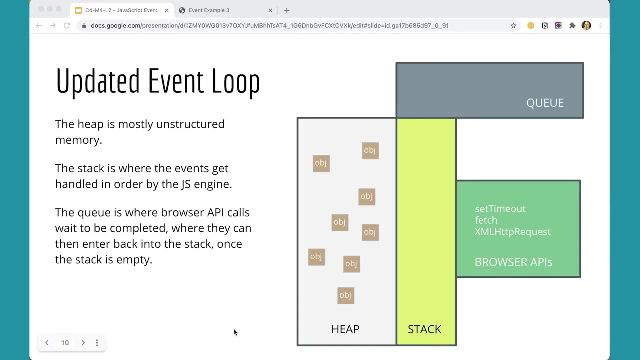 it's going to continue on with the loop. It might be helpful to visualize the event loop in a slightly different way, So that's what I have going on over here. We can think of the heap as being mostly unstructured memory. The stack is where events get handled. 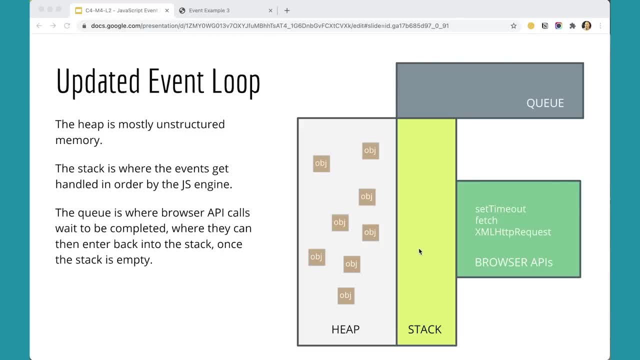 in order by the JavaScript engine. The queue is where the browser API calls are waiting to be completed, where they can then enter the stack back into the stack once the stack is empty, And over here I have some browser APIs that get called at certain times. 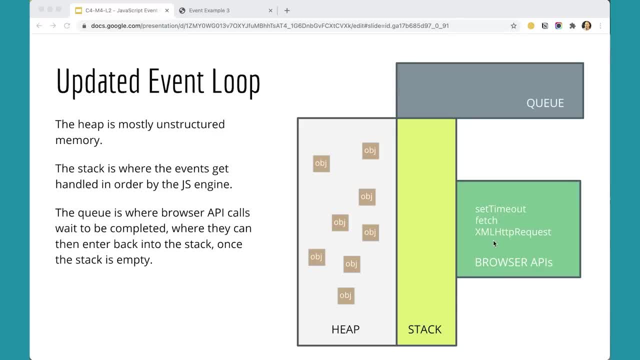 like setTimeout or fetch or the XHTMLHTPRequest object. These are all things that can happen, that take time, And we've already seen all of these in other lessons. So let's go through that example and just sort of see what that looks like here. 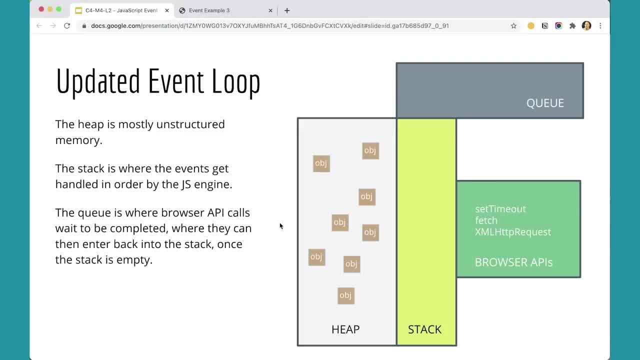 Item 1 enters the stack and it gets processed, because it's just a call to the console log. So it enters the stack, It gets processed, It gets on the console and off it goes. It's done. And then item 2 comes in. 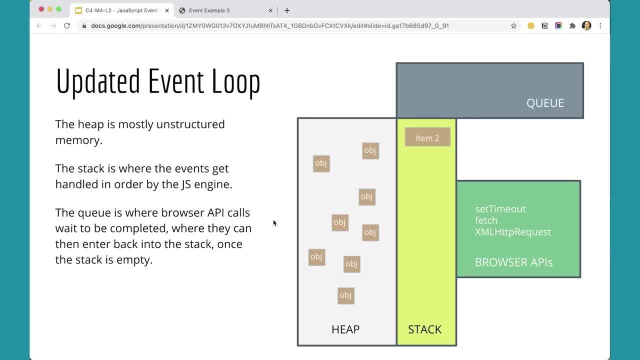 And item 2 says: oh, this is calling setTimeout, So that's a browser API. So it ends up coming off the stack and going over to the browser API where it's recognized as a setTimeout thing, And then it gets sent over to the queue. 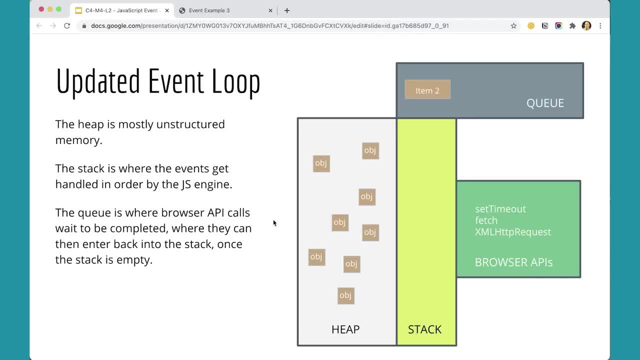 where it's waiting to be finished. It's going to wait those two seconds in the queue and wait to be finished. Meanwhile, item 3 comes onto the stack because it's just a call to console log. It gets processed and it comes off the stack. 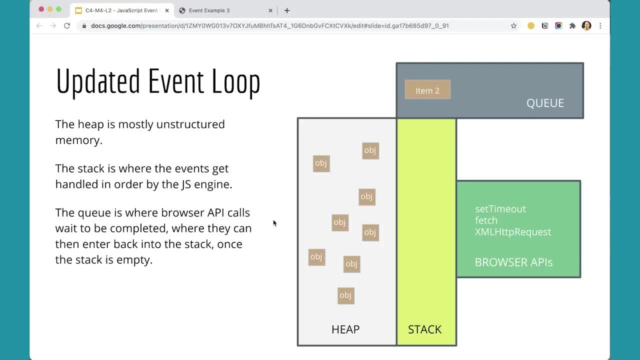 It's done, And then item 2,, once it's waited its full two seconds, it comes back onto the stack where it then is processed and the loop runs and everything gets printed out, And then, when it's done, it comes off the stack. 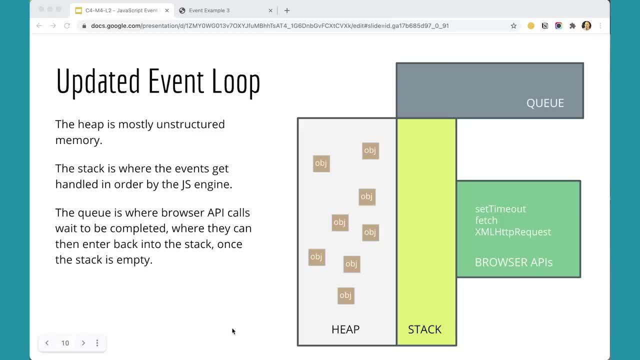 Hopefully that helps you with visualizing how JavaScript actually processes things. Things get put into the stack and taken out of the stack in the order in which they're put into the stack, And the stack can only do one thing at a time, and it does it completely. 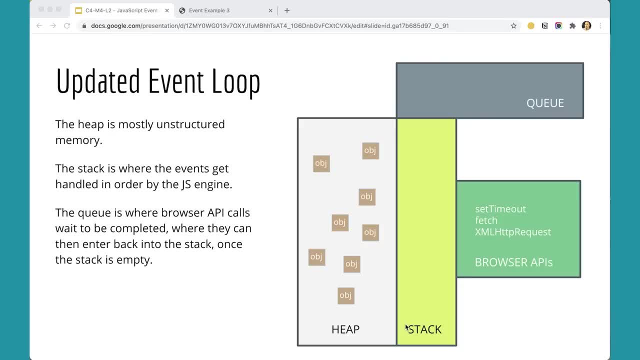 until it's done. If you have something that's making use of a browser API that's going to take some time, then it can get shuffled off into the queue where it can wait until it's done, and then it'll enter back into the stack. 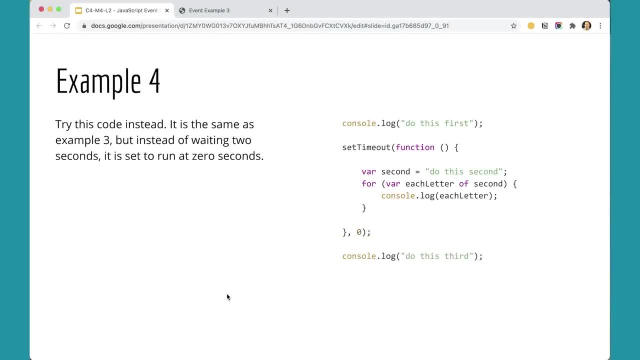 Now this is interesting. Let's take a look at example 4.. And it's got this code here and it's exactly the same as example 3, except, instead of waiting two seconds, setTimeout is set to zero seconds. So let's give this a try. 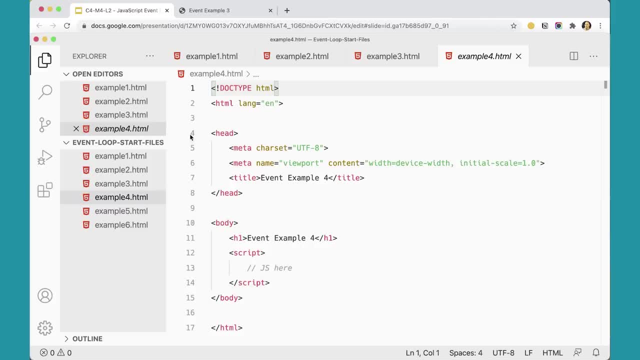 and see what happens If I come over to the code editor. I'm just going to copy what I have in example 3, and I've actually already copied it, so it's in my clipboard And I'm just going to paste it here because it's the same. 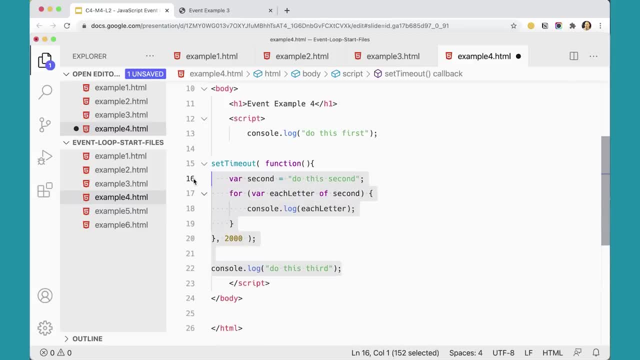 The only thing that's really different here: tab that in Oops too much. The only thing that's really different here is I'm going to set this to zero seconds and save that. So now, if I test this, come over and see what this does. 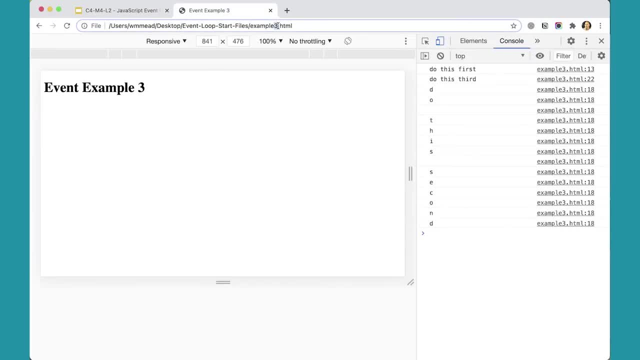 If I come over here and change this to example 4.. Notice it doesn't wait two seconds, but it still runs the first thing first and it's still going to the third thing second and setTimeout, even though it's set to zero seconds. 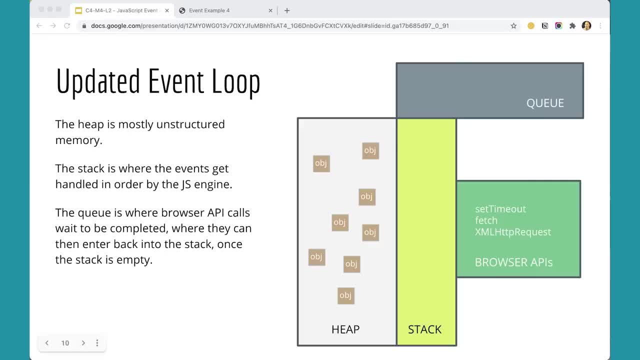 it runs last. The reason why that's happening is that, even with example 4, even with it set to zero seconds, item 1 is coming in here and it's getting processed and then put off the stack. Item 2 comes in and because it's using setTimeout. 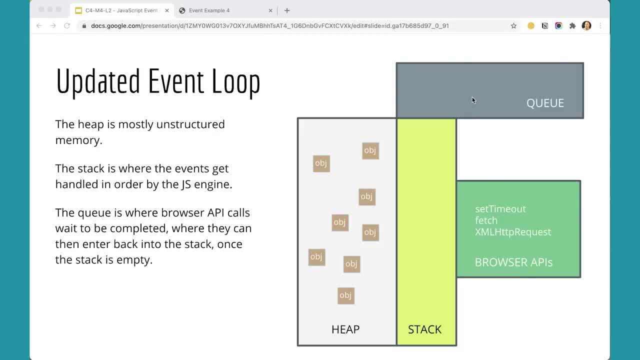 it's being sent to the queue And even though it's set to zero seconds, it's still going through this process of going to the queue And meanwhile item 3 has gone into the stack and come out again before item 2 can make it out of the queue. 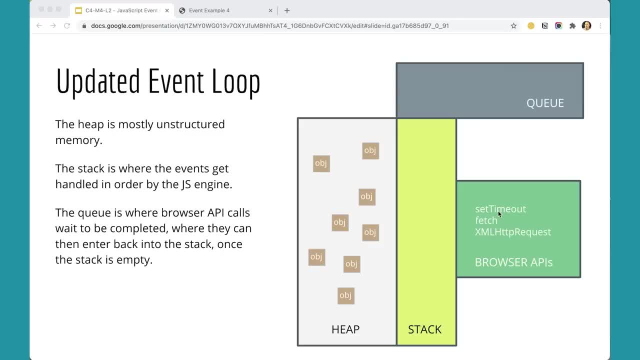 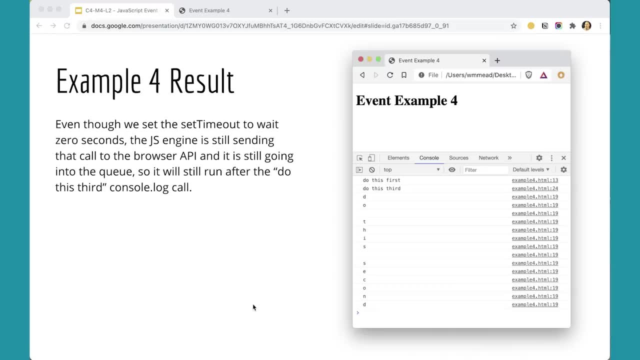 and into the stack. So, because I'm using setTimeout, it's still being processed last. The important lesson here is that setTimeout will wait at least the amount of time that you've set it to wait, but it could take longer depending on what else is in the queue. 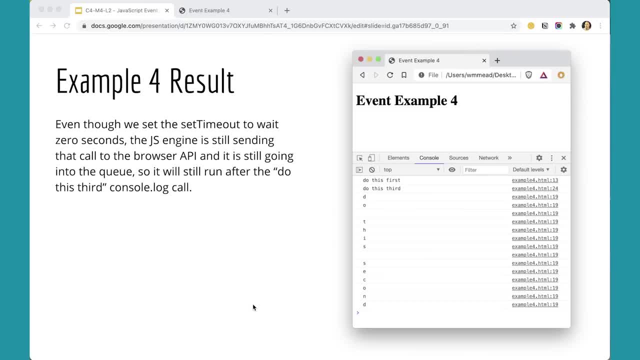 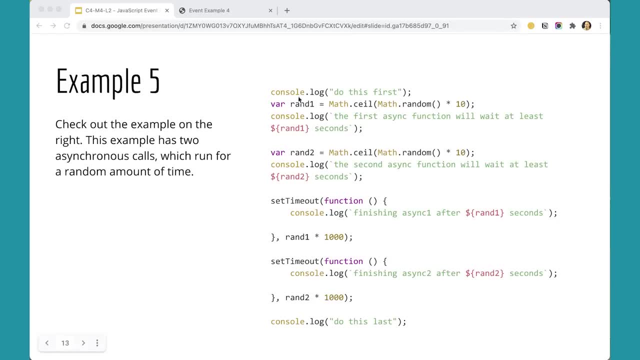 and what else is waiting and what order things are going in. Let's take a look at example 5.. I've got a console log that just says: do this first. That's fine. And then I've got a variable holding called random1. 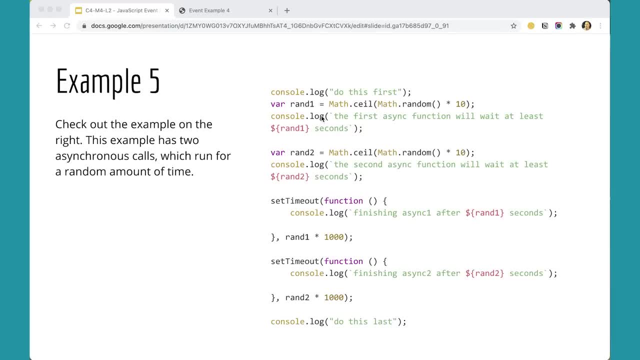 that's holding a random number between 1 and 10.. And I've got a console log that's going to console log out. whatever that variable, whatever that number is, The first async function will wait at least however long that is in seconds. 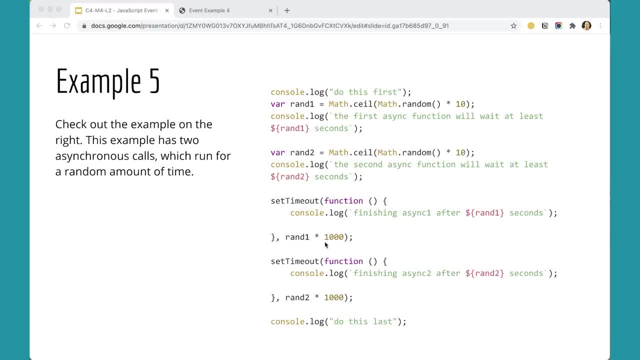 And then I've got random2 that does the same thing. Then I've got two setTimeouts that are each going to run however long. these seconds are random1 times 1,000. So if I pull up a 5 here, it's going to do 5 times 1,000. 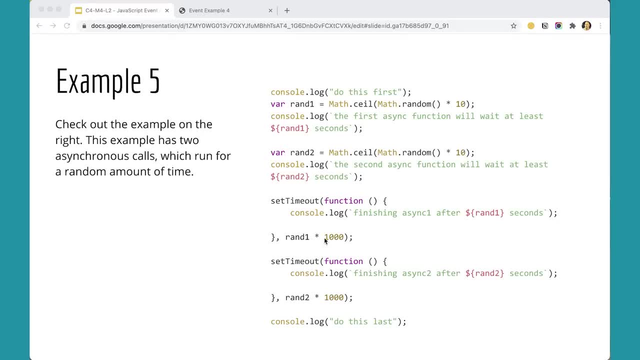 So it's going to give me a 5,000,, which is 5,000 milliseconds. It's going to be 5 seconds. If I pull up a 3, then it's- you know something like that. So that hopefully makes sense. 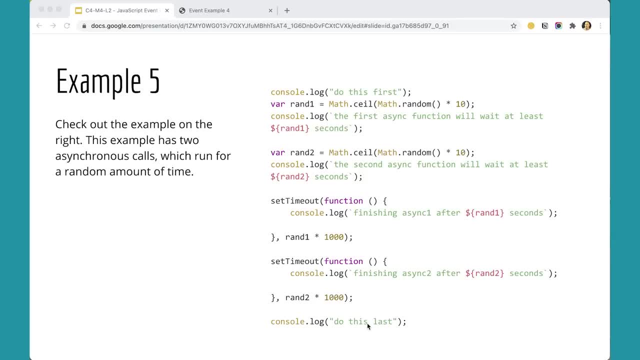 And then, finally, I've got a console log that says: do this last, So let's go ahead and add this into our code, for example 5.. And I really recommend you try this out and you work with the code and see what it does here. 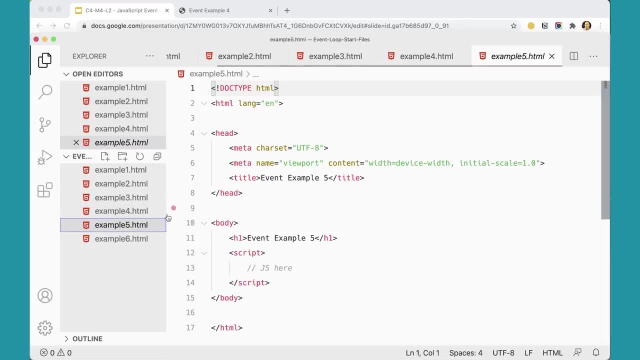 So I'm going to come over here. I'm going to open up example 5. And down here I'm going to have to. I'm going to paste this in here, but you're going to have to type it First. I'll add. 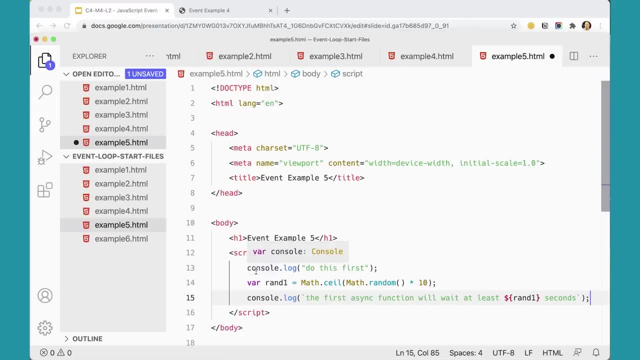 I'm going to get rid of this. I don't really need that comment. I'm going to add the console log. Do this first. Then I'm going to add my variable rand1, which is I'm using the mathco and the random. 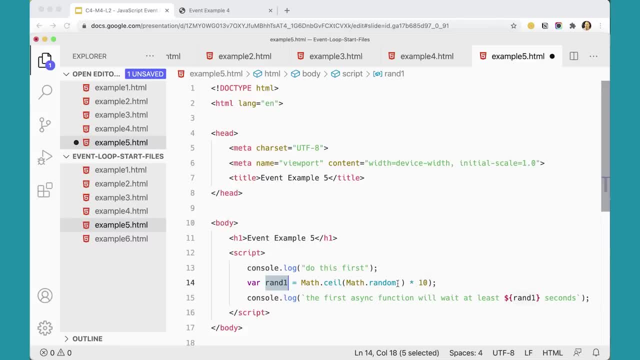 to generate a random number between 1, between 0 and well, actually, yeah, between 1 and 10, I think it should give me, And then I'm going to console log out that first random number there. Then I'm going to do the same thing. 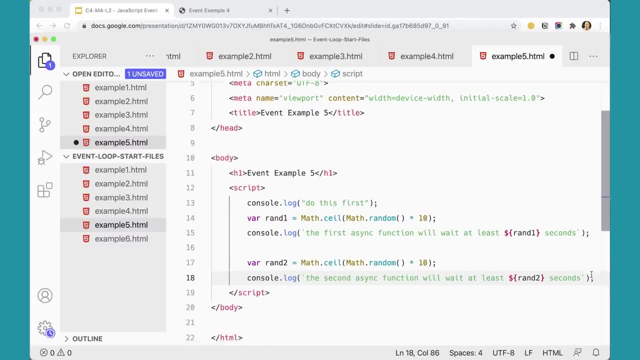 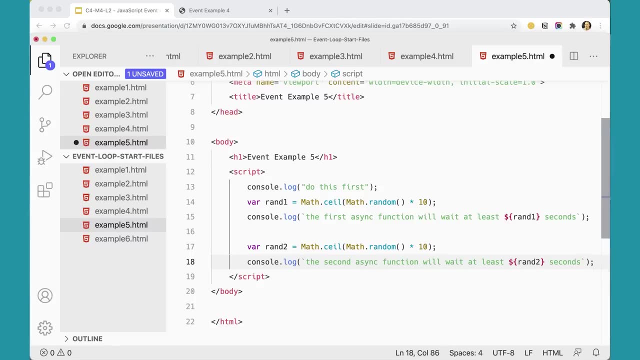 for the second random number, like so. So it generates a second random number, And then I'm going to add a setTimeout, setTimeout, And setTimeout is going to run a function for a period of time, And I'm going to do it whatever rand1 is. 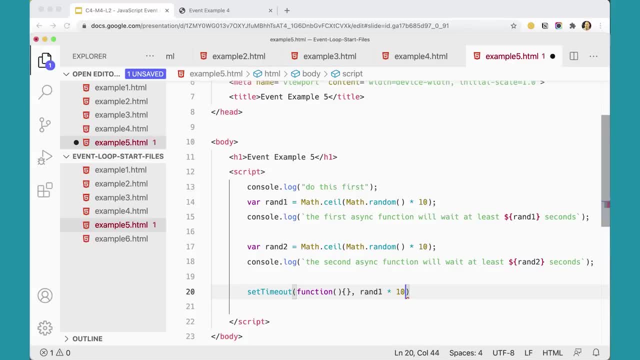 times 1000.. 1000, not 10,000.. There we go. So now I've got my setTimeout, And what am I going to do in this function? I'm basically just going to console log out, finishing async1 after random 1 seconds. 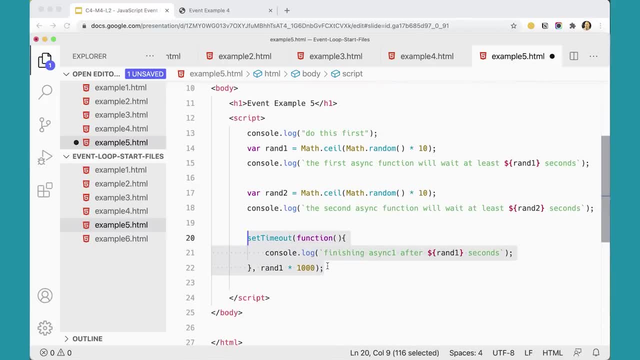 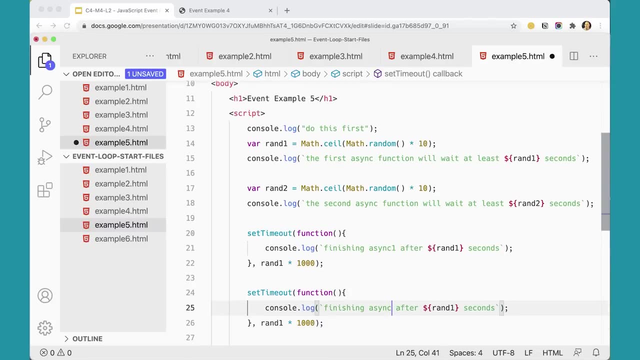 And I can actually copy this And do the second one from it, Because this one's really just going to be async2 after rand2 seconds And then down here rand2.. Make sure you fix it in all of those places. And then finally, 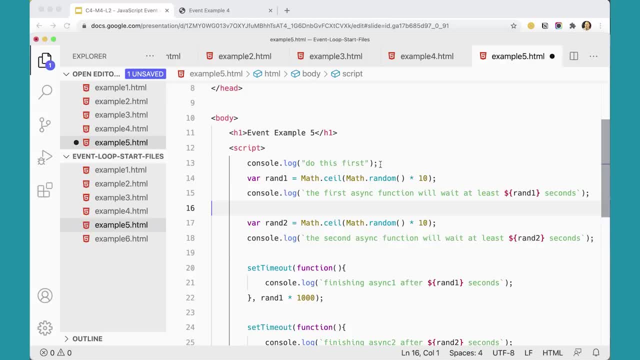 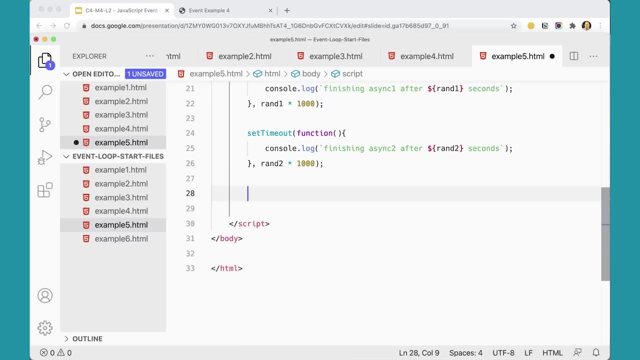 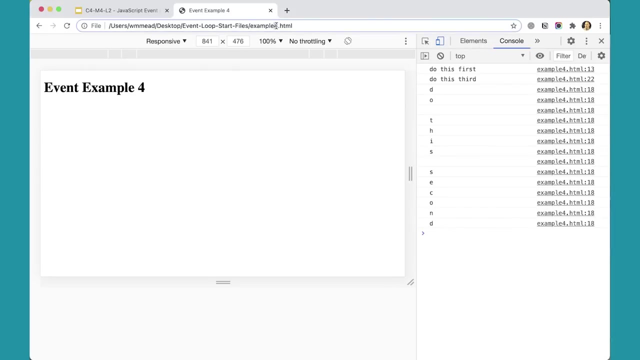 I just have a console log that says: do this last, Copy this one and stick it down here. Do this last, Make sure you save the file. And then I'm going to come over to my browser And let's run this a few times just to see what happens here. 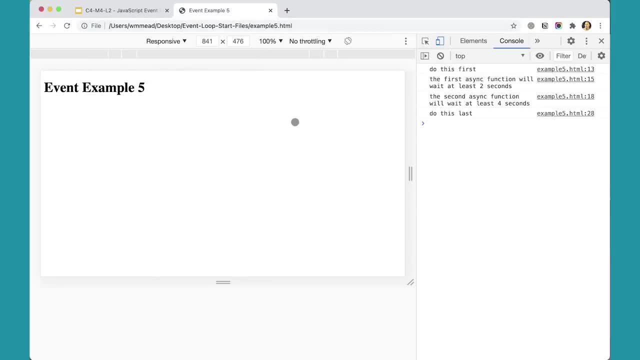 Change this to example 5. And you can see that. okay, do this first rand. The first function will wait at least 2 seconds. The second function will wait at least 4 seconds. Then do this: last fired And then the two asynchronous functions actually ran. 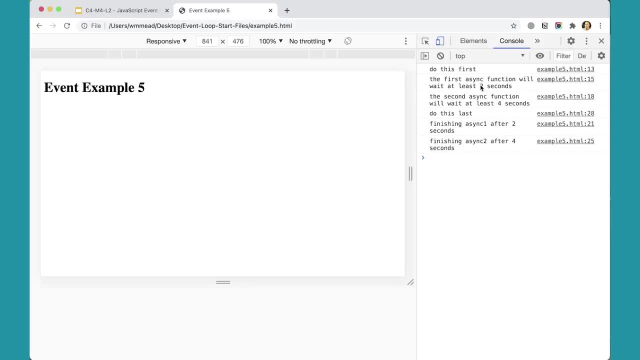 after 2 seconds and 4 seconds, And you can see that the first one ran first 2 seconds And the second one ran second after 4 seconds. Let's refresh it. So now the first one's going to go 9 seconds. 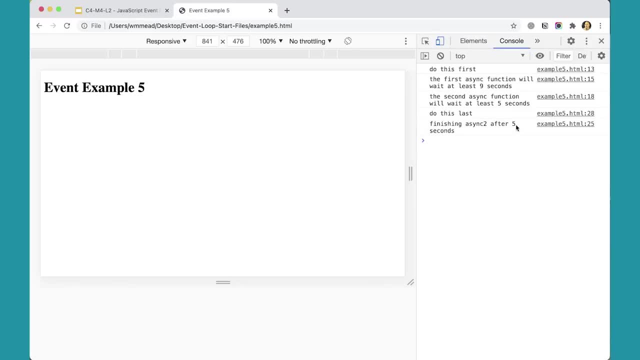 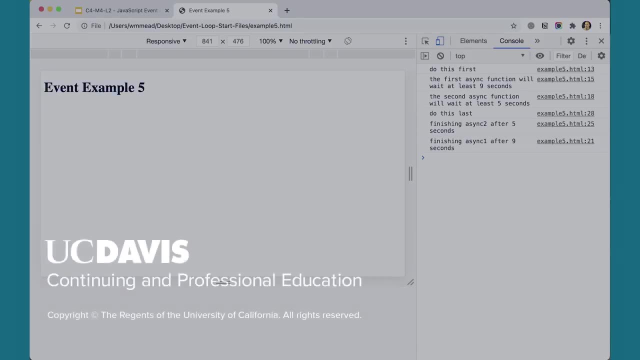 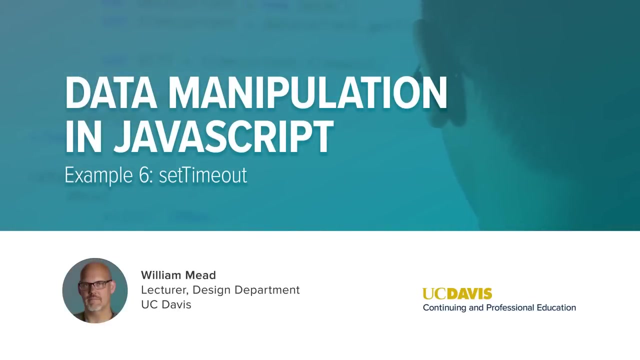 And the second one's going to go 5 seconds. So you can see that the second one ran first 2 seconds. So you can see that the second one finished first And then the first one finished last. So that's pretty interesting. 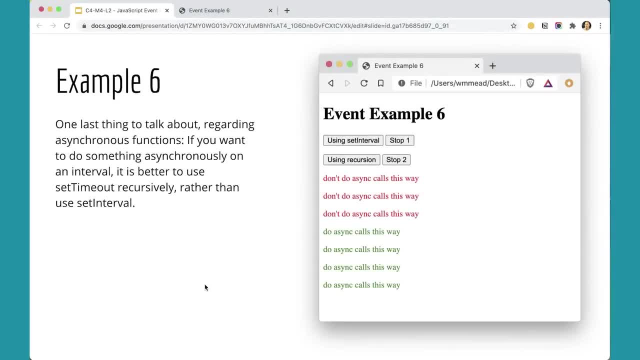 Example 6.. One last thing to talk about regarding asynchronous functions. If you want to do something asynchronously on an interval, it's better to use setTimeout recursively than to use setInterval. We've looked at setTimeout and setInterval in the past And you know that setInterval runs at a particular interval. 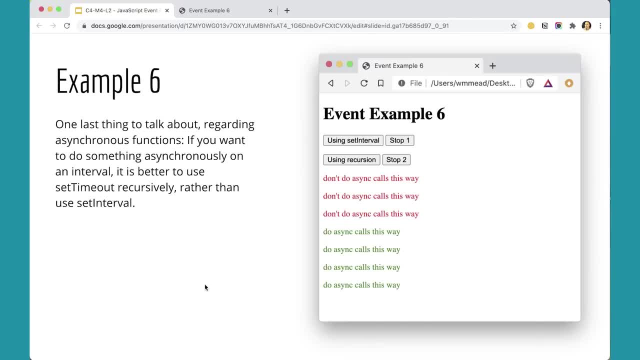 We've also talked about recursion, And recursion is very powerful And it allows you to run something, have a function call itself, basically after a certain amount of time, And the reason why that's better, and you can open up Example 6 and try this for yourself. 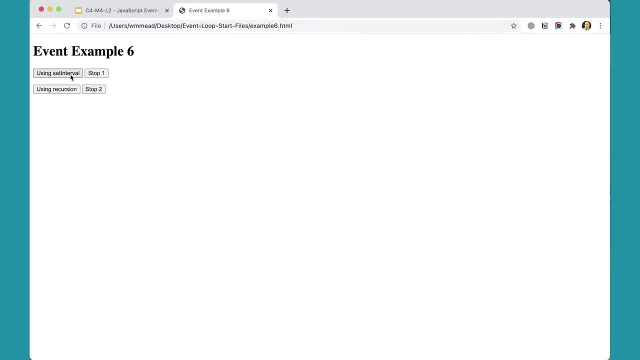 And we aren't actually doing anything, anything asynchronously here, But it's sort of simulating it. So this is running this thing on setInterval, whereas this one is using recursion, And I can stop both of them. And what's the difference here? 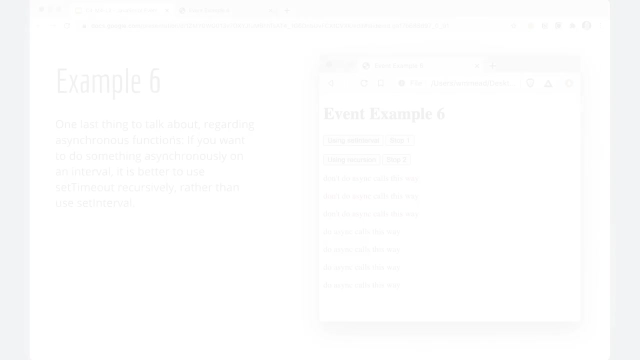 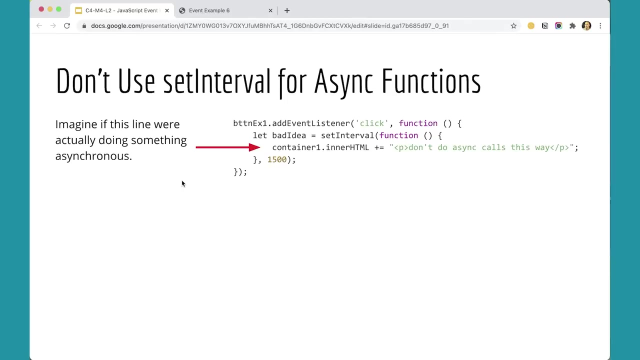 What's the difference between these two scripts? Imagine so, here we're using setInterval. But imagine this line: here the thing that we're actually doing is an asynchronous function. So setInterval is going to run every 1500 milliseconds, or 15 seconds, no matter what. 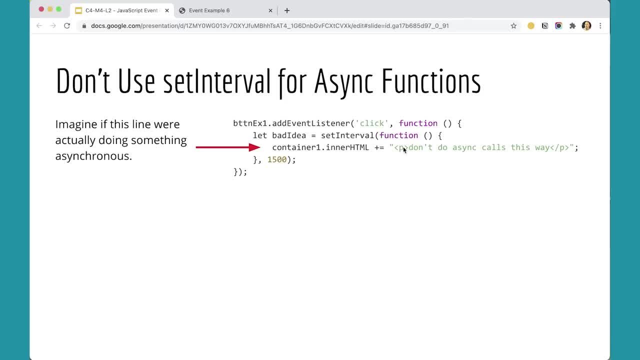 But if this thing were to take longer than 15 seconds to complete, then we'd start running into problems. So that's why it's not a good idea to use setInterval with an asynchronous function, because we don't know how long this is going to take. 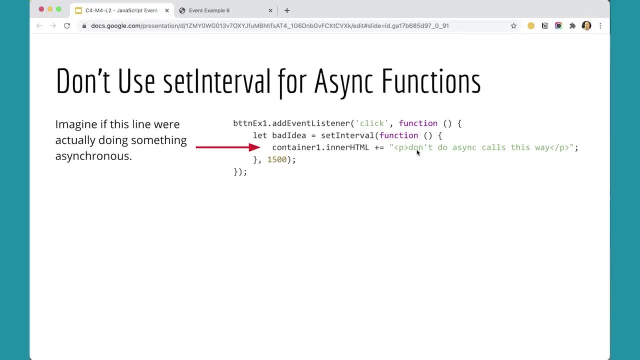 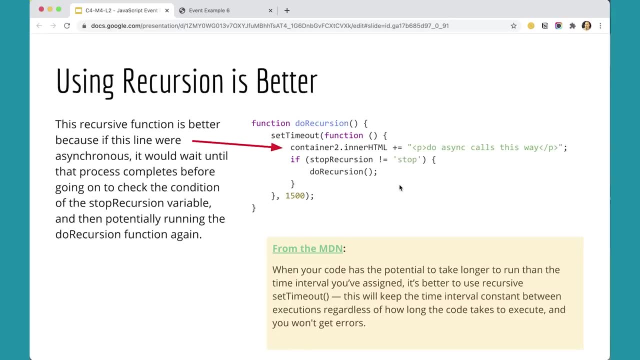 In reality, here we're just putting a paragraph on the page, So that's probably fine to use with setInterval, And what you should do instead is use setTimeout to say: we're going to run this every 15,. we're going to run this for 15,. 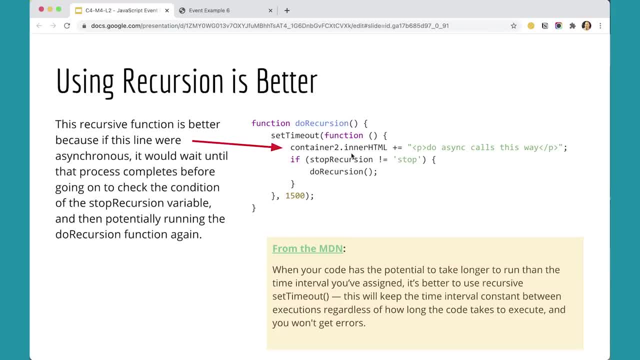 we're going to wait 1500 milliseconds to run this And then, when it does it, it's going to do its asynchronous thing. So this is asynchronous. And then, when you know, if we're not telling it to stop, it's going to do recursion again. 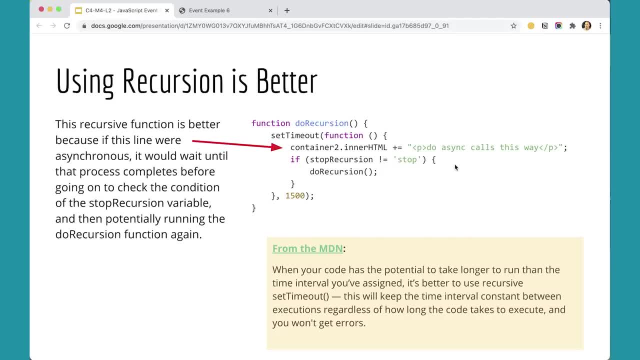 But it's only going to do this after it's completed its asynchronous function here. So it's much better to do asynchronous calls using recursion if you want to do something on an interval instead of using setInterval. And down here I have. this is listed right from the MDN. 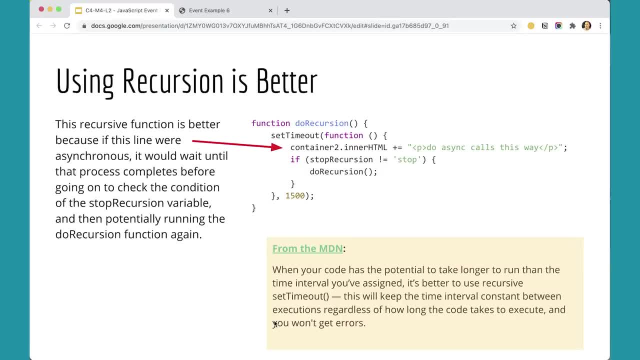 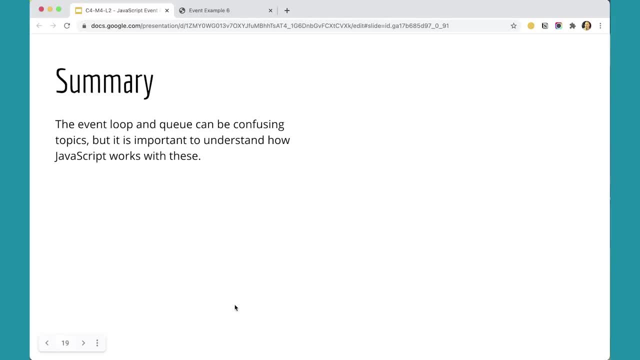 specifically about doing this, And so this is what they're advocating on the MDN as well. In summary, the event loop and the queue can be confusing topics, but it's really important to understand how JavaScript works with these elements of the system that it has built into it. 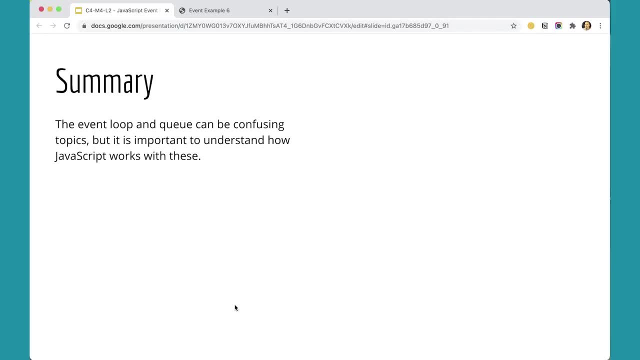 There are some really great YouTube videos out there that explain it. Some of them are a bit older, but you might try looking to YouTube to finding some other good examples of people talking about this if you're still feeling a little bit confused about it. 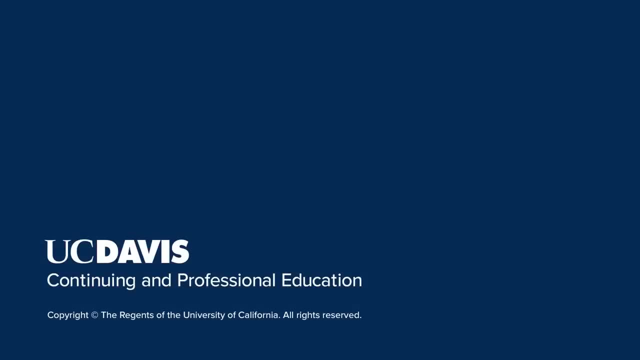 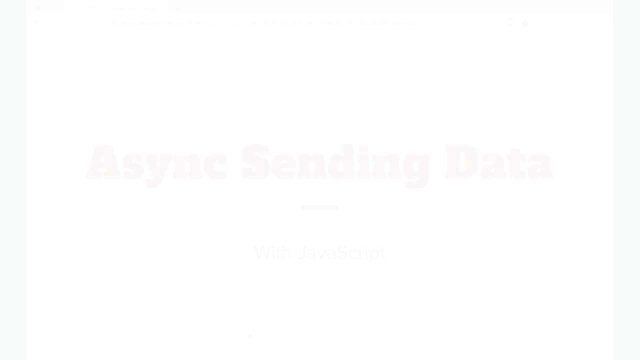 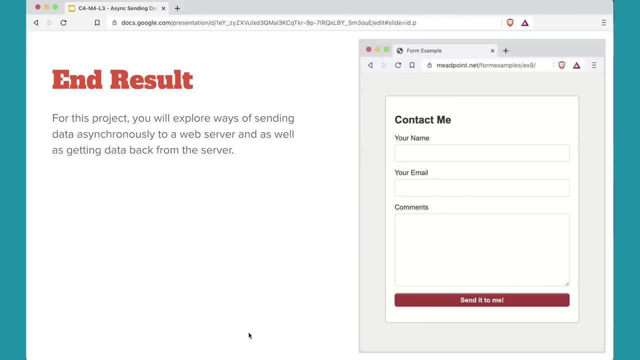 But hopefully these examples have really helped Asynchronously sending data with JavaScript. For the end result of this project, you're going to end up with a really nice email contact form that you could use on any website, And it's going to send data asynchronously. 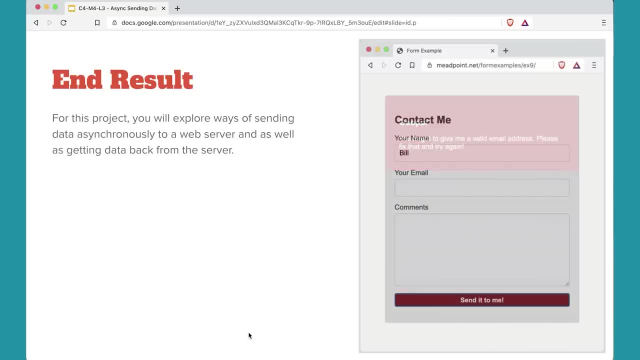 to a form processor that will process the form Plus. it'll have some nice validation built in and a nice interface built in so that if users don't fill out the form properly it won't work, But when the data goes through you get this kind of nice spinny effect. 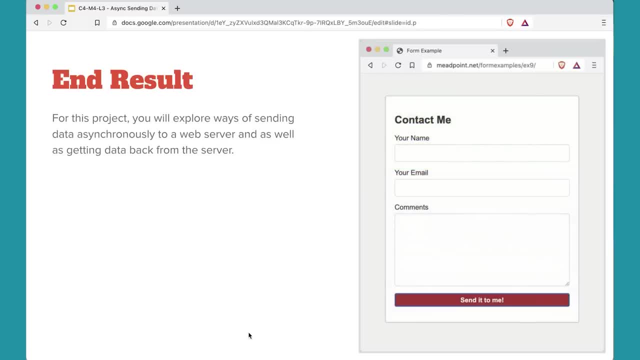 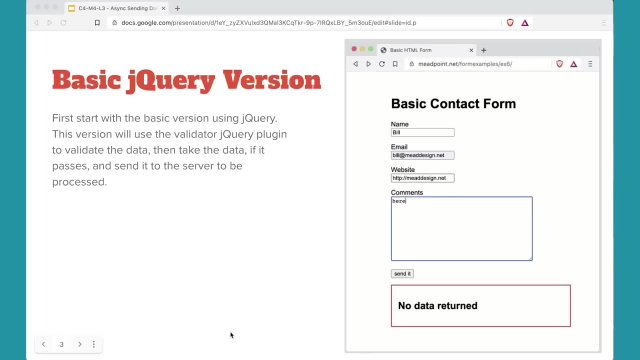 and then a nice success message at the end of it. So I think that'll be really fun and it's really useful And I think you'll like it. when we get to the end here, We'll start our project with this. We'll start our project by making a basic jQuery version. 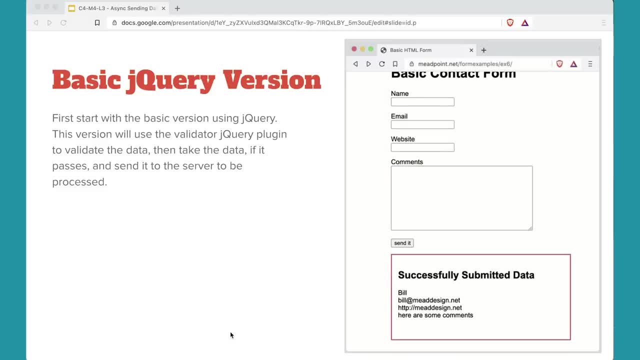 that allows you to see how we can send and receive data to the server. Before we did some work where we were actually just receiving some data, but now we're actually going to send data to the server as well. So that's pretty interesting and kind of fun. 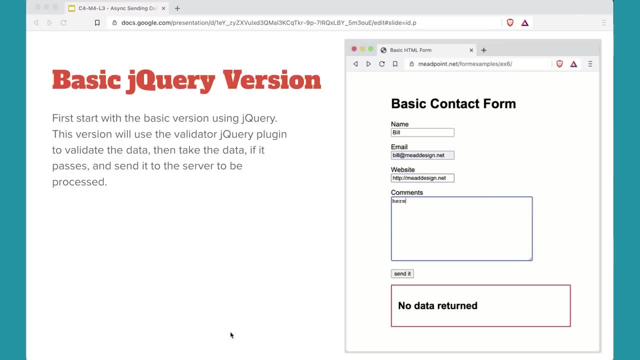 In this case, the server's just sending back the data that we sent to it, so it's nothing too exciting, But by the end we'll have the nice contact form, So let's get started on this. Switch to the code editor. 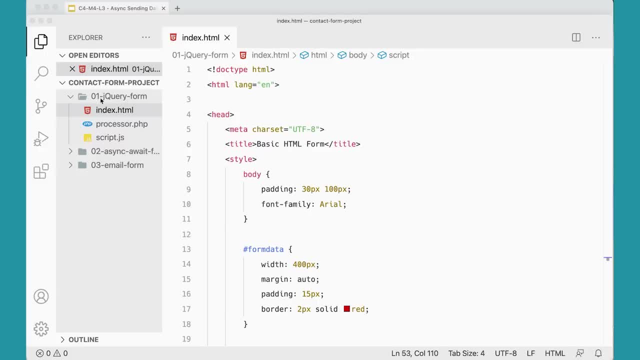 and you'll see, I have inside my jQuery form, my 01 folder here, 01 jQuery form folder. I have an index file and it's just a basic index file, basic HTML file with a little bit of styling, not very much. 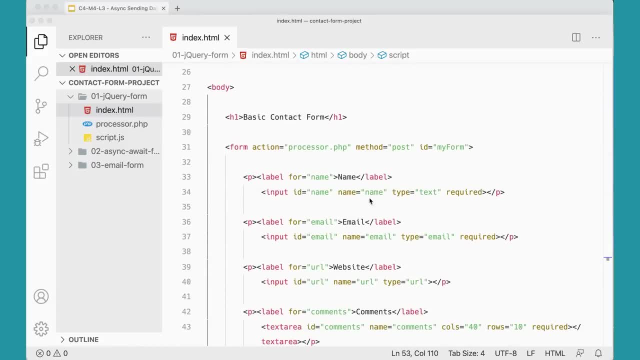 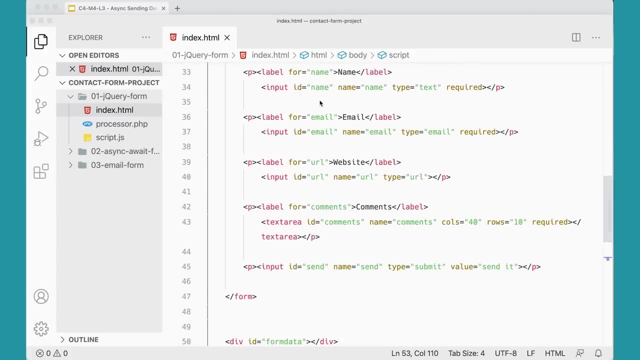 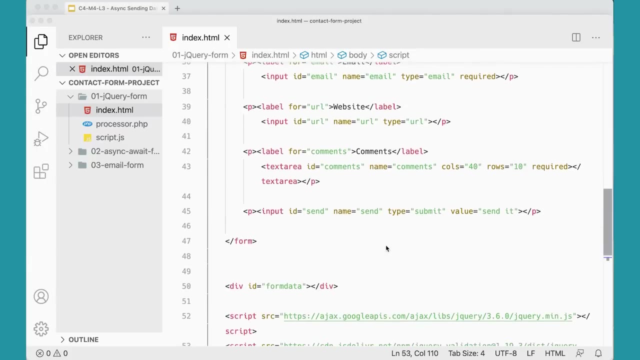 and a form on the page- basic contact form- with some text view, some type yeah text fields, an email field, a URL field and a text area and a send button Down here. you'll notice that I have jQuery plugged in. 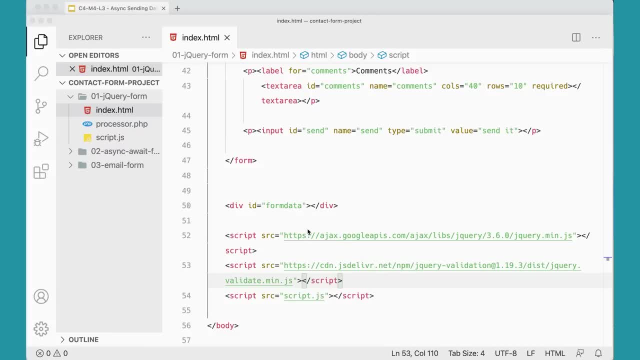 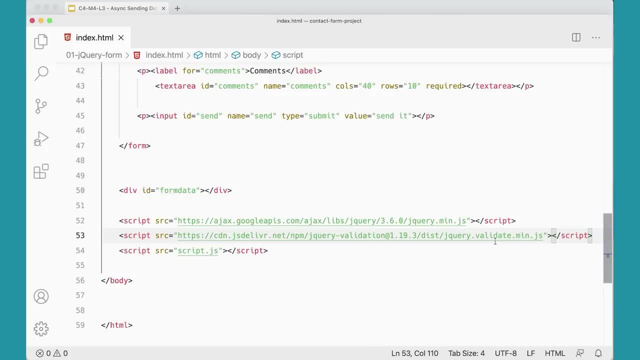 the 3.6 version which, as of this recording, is the latest version of jQuery. I also have the validator plug-in added, so we'll use the validator plug-in to validate our script. And then I have a link to my jQuery. 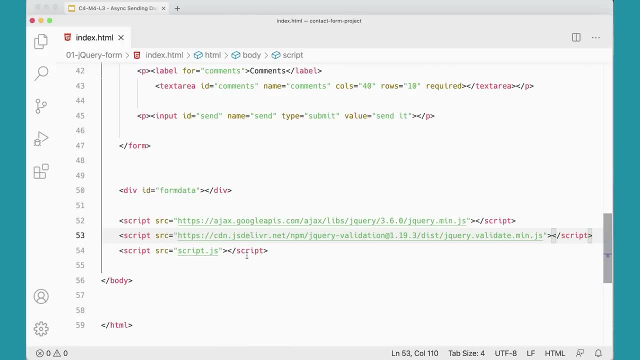 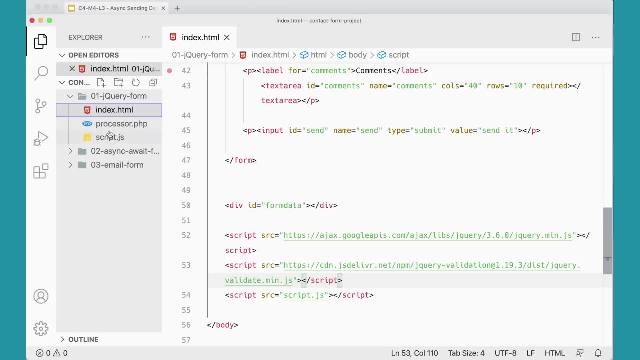 and my own JavaScript file. So we've got all of that in place and ready to go. The next thing we should look at really quickly is the PHP file. So if you come over here and look at the PHP file, it's pretty basic. 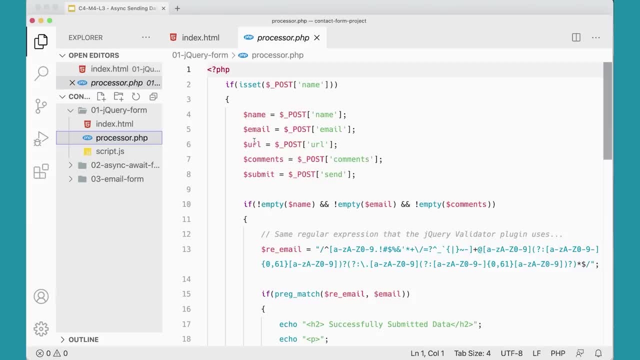 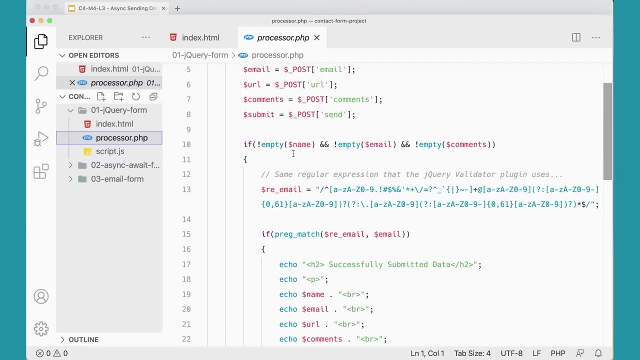 I'm just checking to see if the data's been sent. if it has, I'm attaching it to local variables and then I'm checking to. I'm just doing some basic validation on the backend, as we've talked about in a previous lesson. 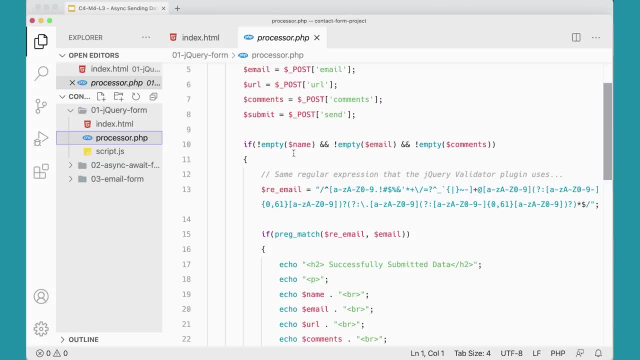 to that. it's really important to make sure that on the backend you're validating your data as well as on the front end. So I'm just checking to make sure that the name field, the email field and the comments field are empty. 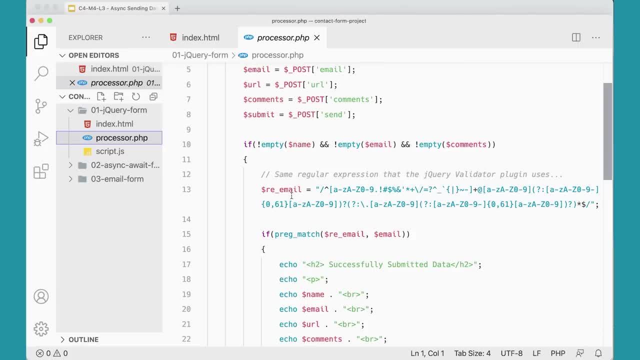 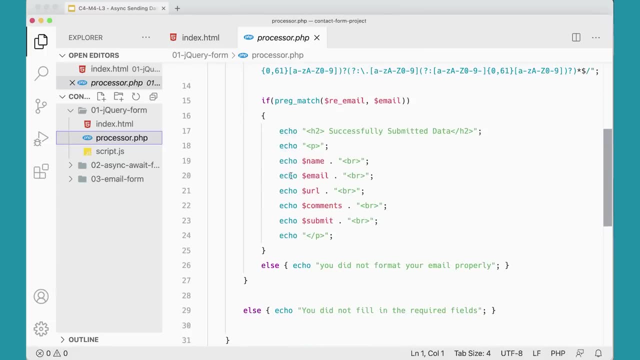 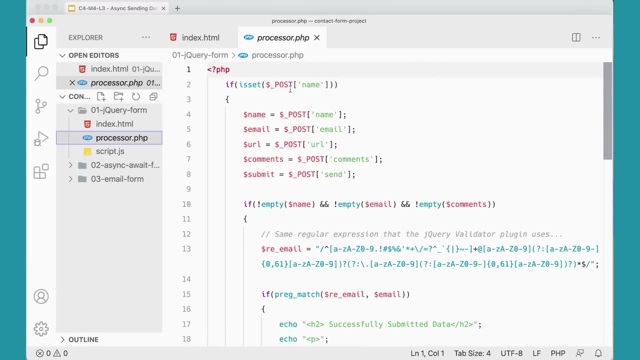 I'm also checking that somebody typed a valid email address into the email field using the preg match method And then I'm just echoing out these fields. Now, one thing that's kind of important to note here is that if nothing is being sent to this form at all, 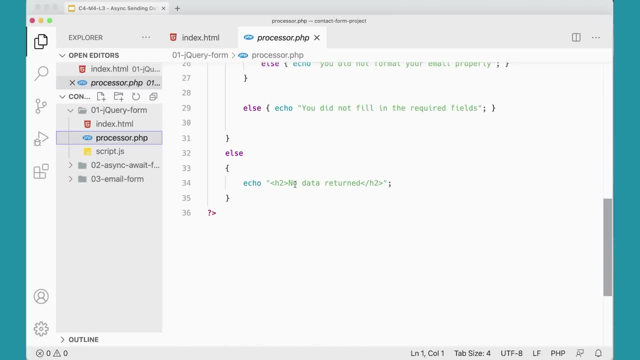 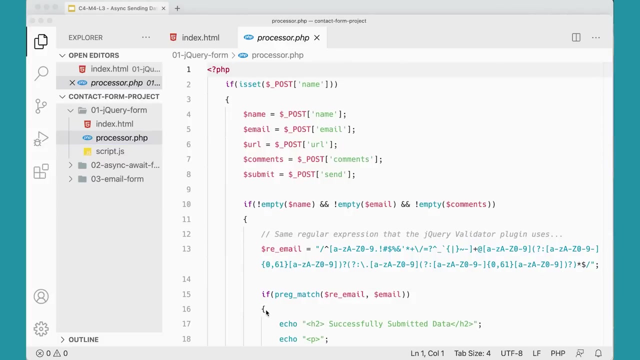 it's going to echo out an H2 that says no data returned. So if I load this page up in my browser now, I should be getting no data returned Once we add just a little bit of JavaScript to connect to this file. Now I should also add that these folders: 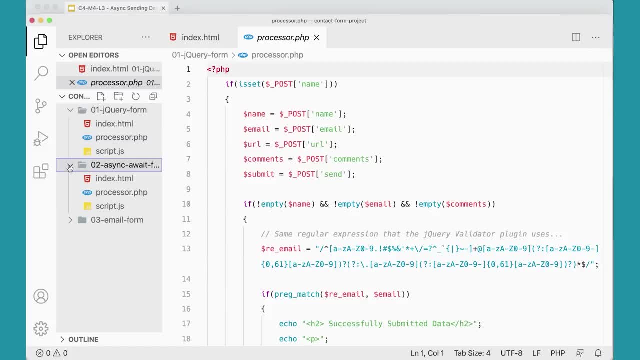 have the processor PHP file in them. This one has it. This one has the exact same file. This is just the same file, Just a copy of that one. And then down here this one's a little bit different- the PHP file of your email processor. 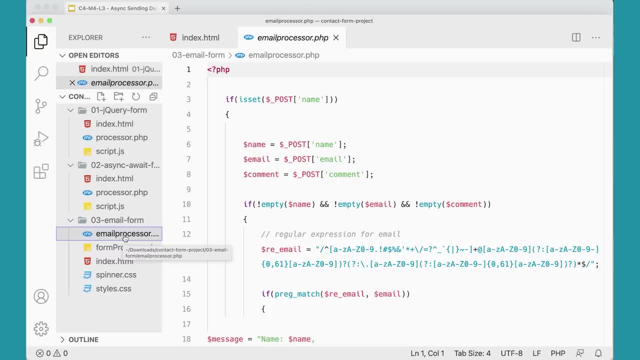 And we'll look at that one when we get to this part of the lesson, But we don't need to use these files. I'm including them here for you in case you want to refer to them, But I actually have these files on the server. 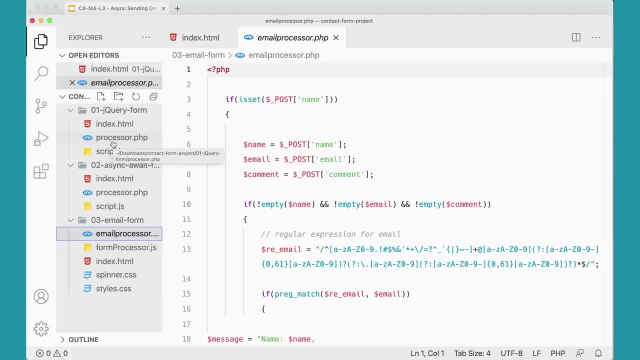 that we can use to remotely access. Otherwise, you would need to to do these projects. you would need to put these projects on some sort of server, either local host- you could use MAMP or XAMPP or one of those- or if you have your own web server. 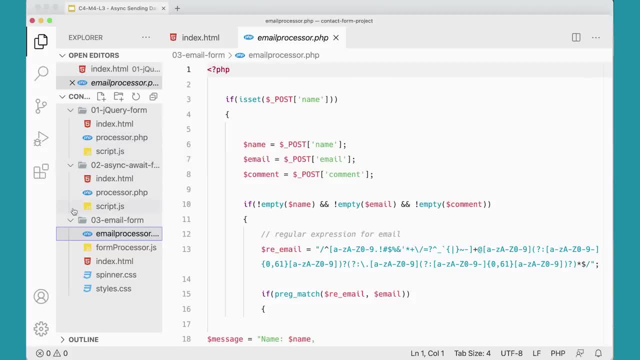 you can put them up, But you don't need to do that because I actually have these PHP files and we can actually access them remotely. So we'll be doing that, Okay, great, That gives us a foundation of where we are for this first part of this project here. 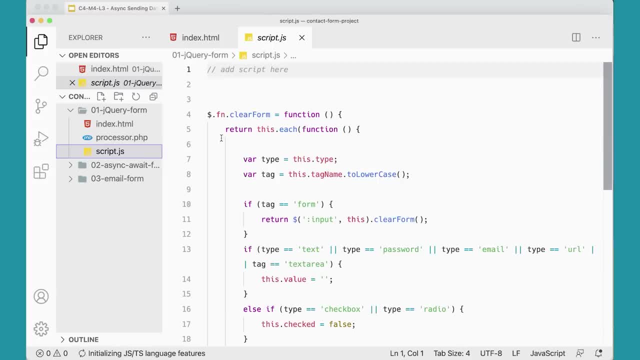 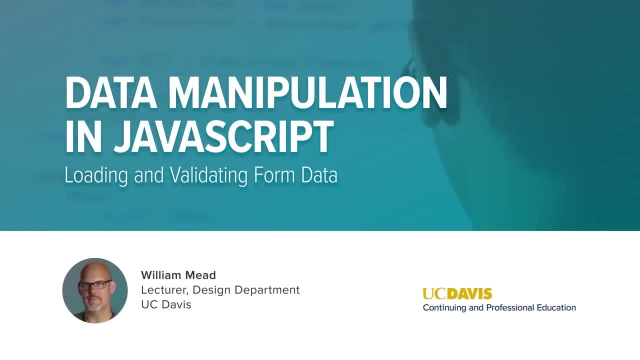 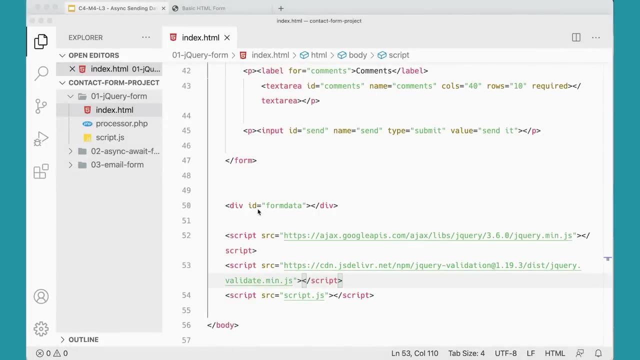 And we'll start working on coding on the script file here in the next video. Okay, so we talked about our files and now we're ready to get started. We've got our Google, our loading from Google, our jQuery libraries loading up, as well as our validation plugin. 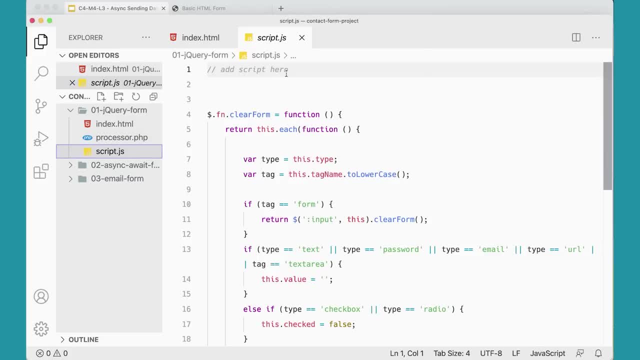 So now we can go over to our script file and start using some jQuery over here. You'll notice, on the script file, I have a function here that's going to be used to clear out the form when we're done, And you can just ignore that for now. 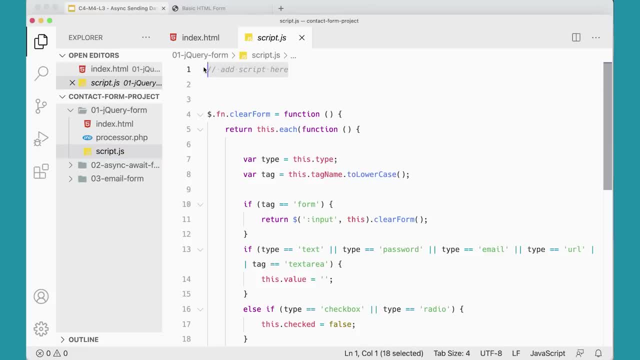 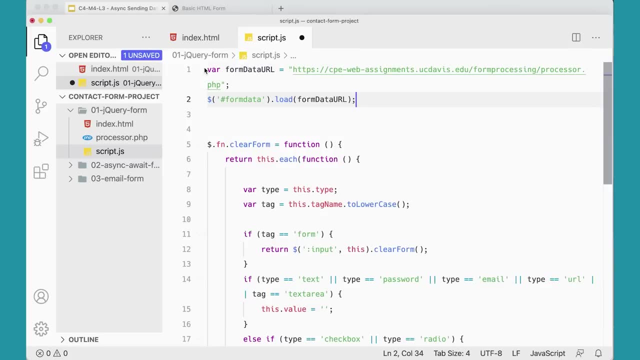 I'll talk about that in a few minutes, But up here I'm just going to add where it says add: here I'll get rid of that comment. I'm just going to add this form data variable here. I'm going to close my Explorer here. 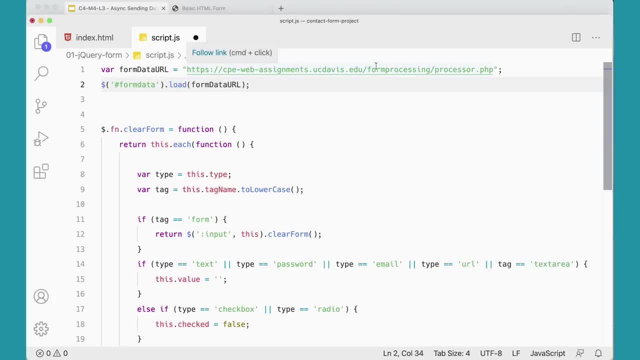 so you can see this a little bit better. And this is just the URL where that processorphp is up on our server here, our CPE web assignments server. So instead of using the one that's locally in the folder, because if I were to do that, 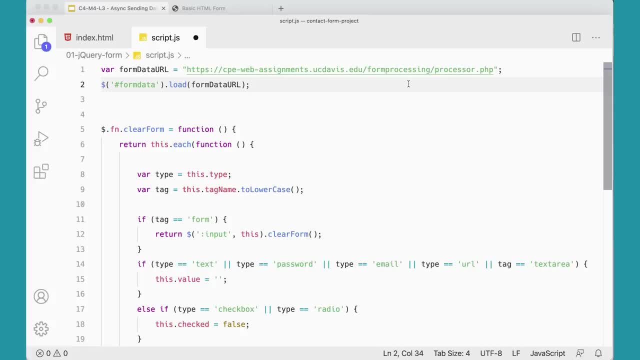 I would have to put this whole project on a web server somewhere or run it through localhost using MAMP or XAMPP or something like that. Instead of doing that, I'm just going to link to this file up on our server And then I'm going to say form data. 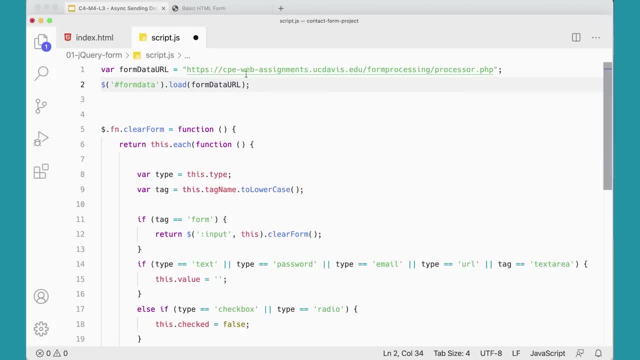 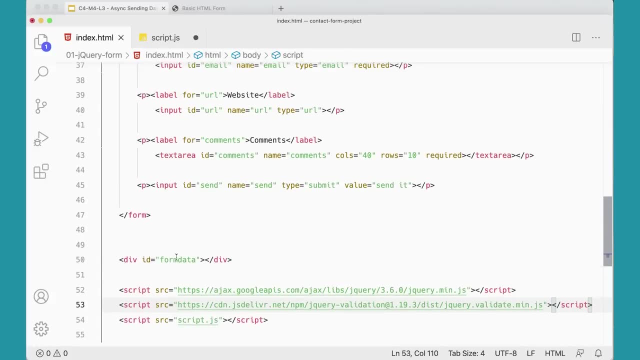 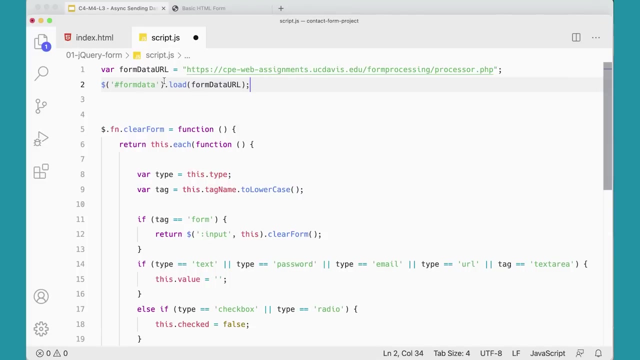 load form data URL. load that file. So that's going to come over and find this element on the page div ID- form data And it's going to load form data URL. It's going to load that file And that file, as we said just a minute ago. 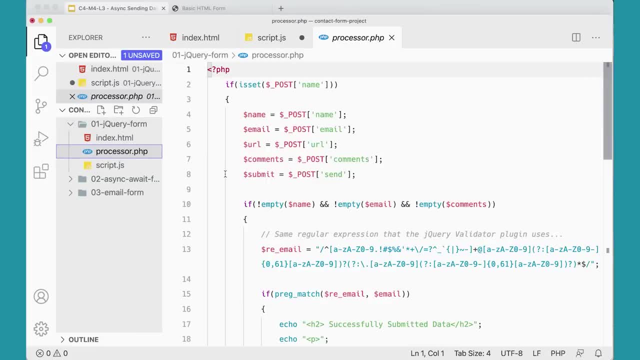 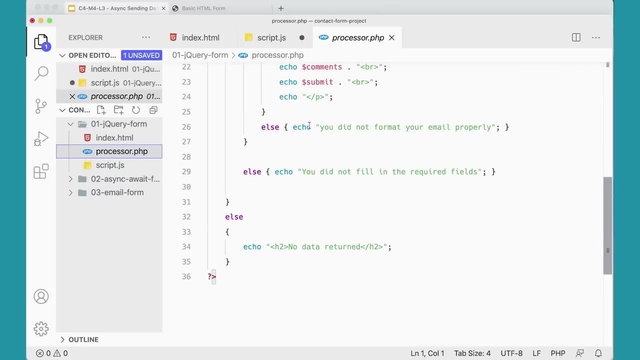 if we haven't actually sent any data to it. all it's going to do is send us something back that says an H2, that says no data returned. So that's what we should be getting now if we test this file out. So I'm going to save that. 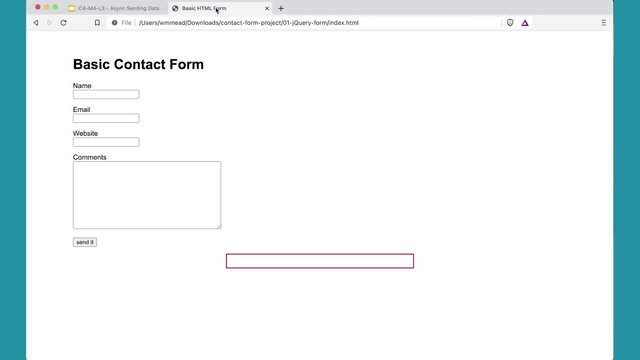 And if I come over here to my browser here and here's my file and it's just loading from my downloads folder here. But if I refresh this, it should go out to that server and load that file And all it's getting back is an H2. 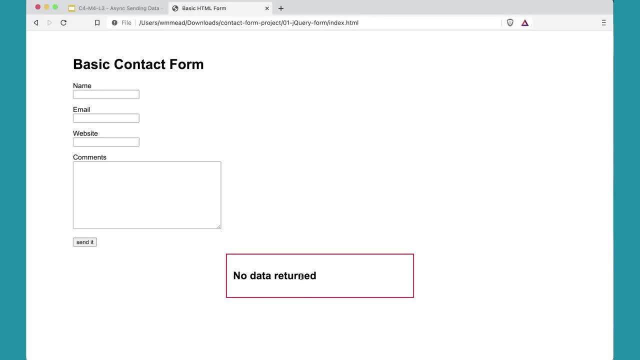 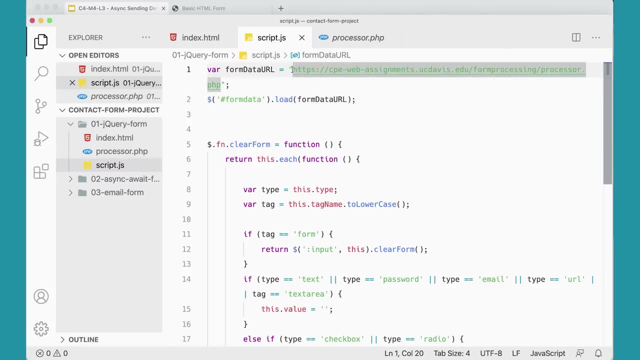 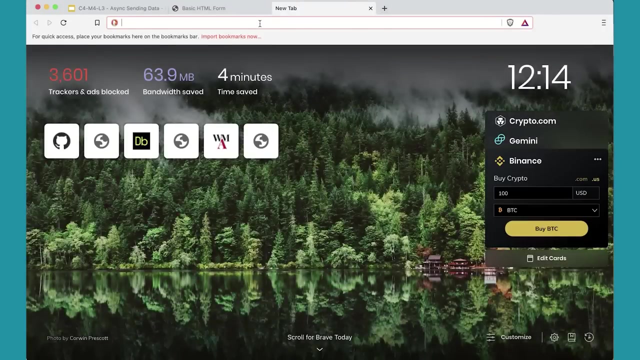 that says no data returned, So that's coming in fine, just fine here. It's interesting to note that if you were to just take this, copy this address, this here and come over and paste it in up here, what would you get back? 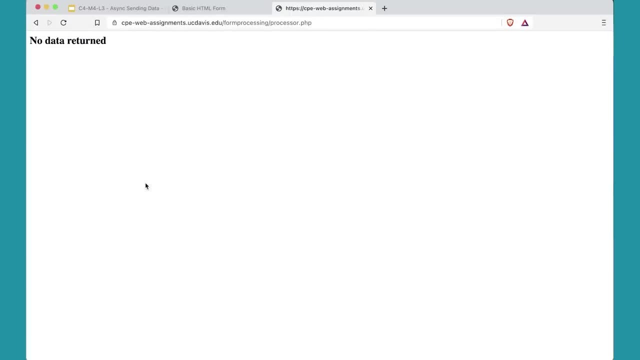 No data returned. And if you view page source on this, it's not a whole web page, It's just an H2.. No data returned. That's all it is. That's all we're getting back. But now that page is actually getting placed. 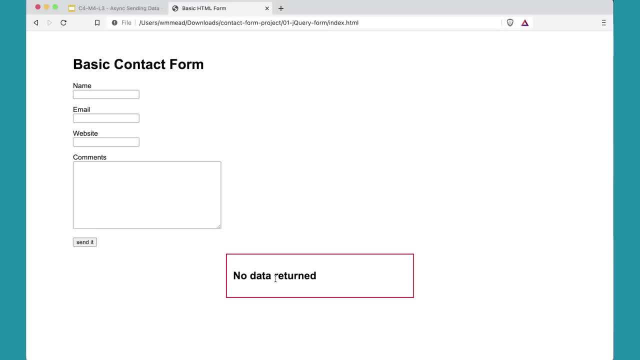 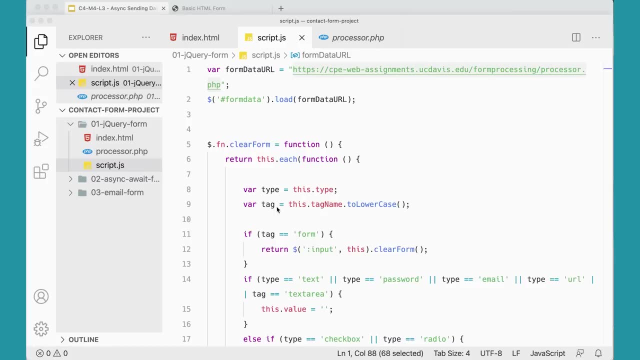 that H2 is getting placed inside this element in this page. So this page is asynchronously getting that file and returning it and sticking it there. Hopefully, you have a good sense of how that's working. I'm going to minimize this And then I'm going to come down here. 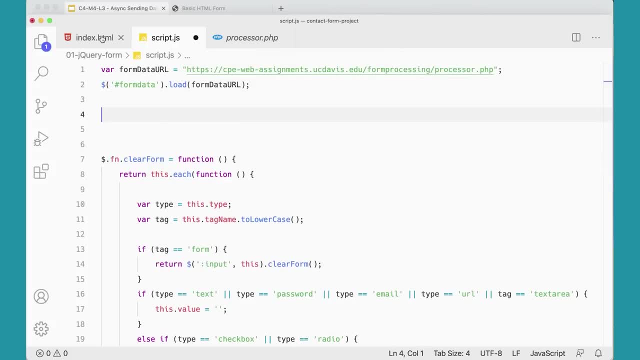 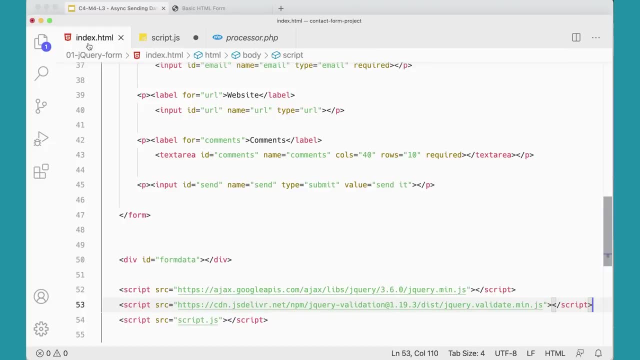 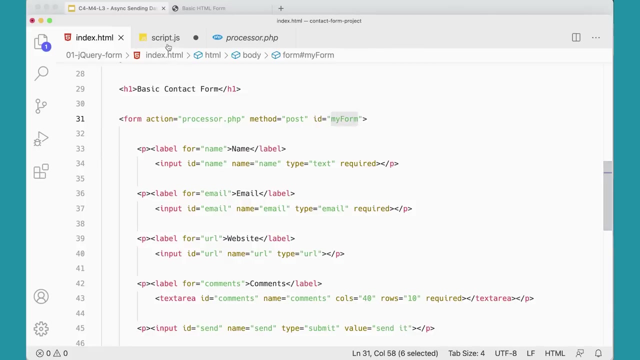 I'm going to start working on my script where I need to get the ID here. First, I'll type my jQuery object here, pound, and I want the ID of the actual form form, my form, this ID here, And I'm going to take that ID here. 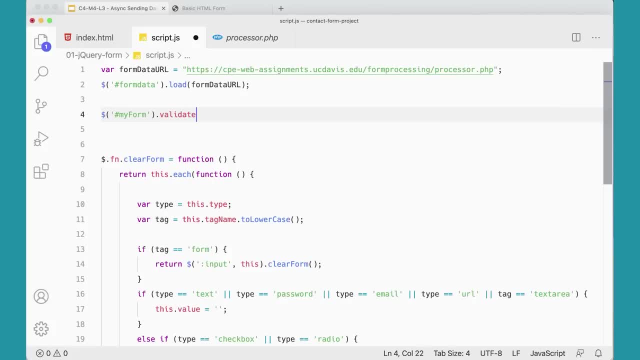 and I want to run the validate function on here. This function is available to me because I've plugged in the Validator plugin and we're just doing the very basic validation of the form. We're not doing anything too fancy here, And then I need an event handler. 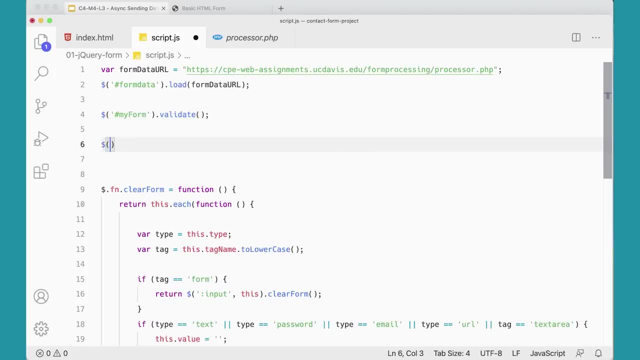 that is going to go and get the same form, pound my form and add a set submit event on there And when we try to submit the form, we're going to run a function like so And we're going to pass in the event. object: 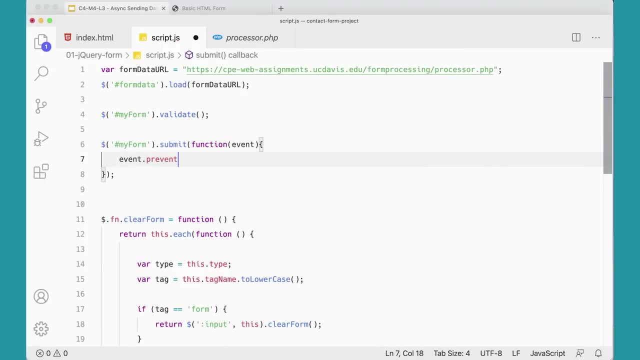 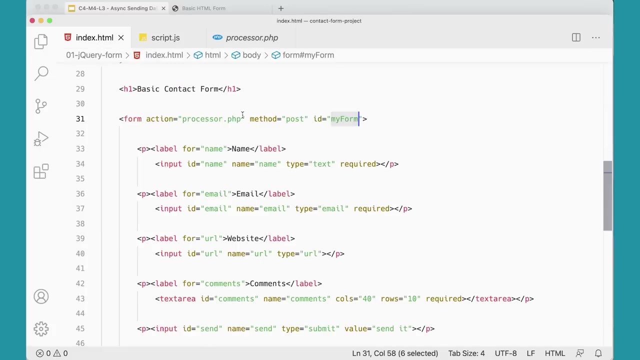 and then do eventpreventDefault So it doesn't actually submit the form. It's kind of interesting to note that over here I do have actionProcessorphp here so that if this were not going, if JavaScript were not going to capture this and keep us from submitting the form, 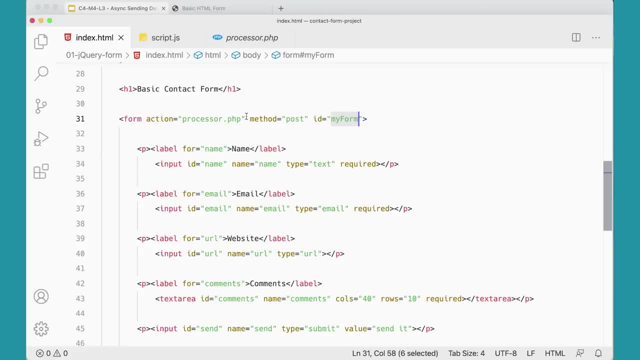 it would actually send you to this processorphp file And you could remove this from here because we're not going to use it at all. But often for progressive enhancements, you actually want a file that you would send people to in case the JavaScript didn't work for some reason. 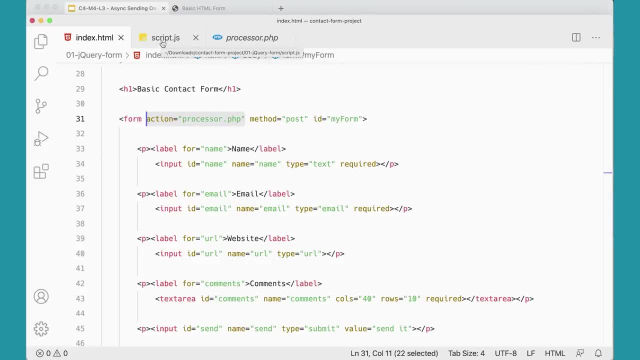 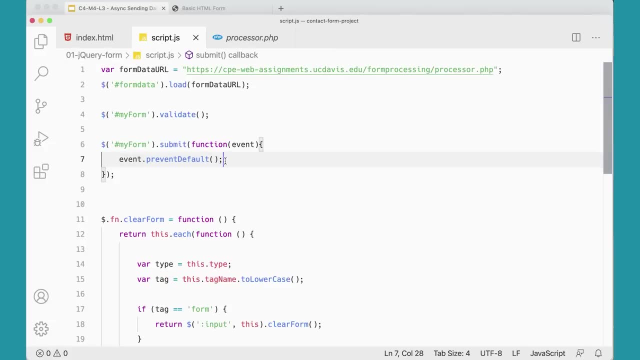 Maybe somebody has it off or something like that. You never know, But in this case you could just delete it. We're going to delete it from there if you wanted to, because we're going to prevent that default action going to that form from coming through. 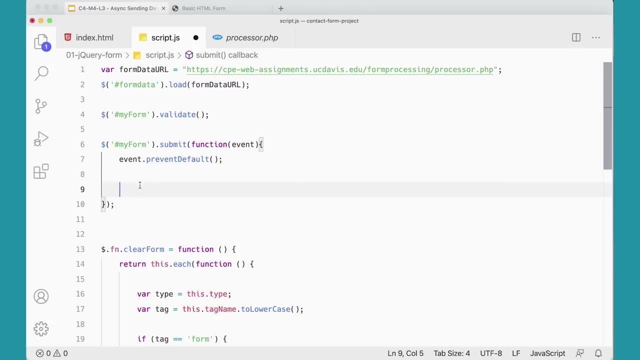 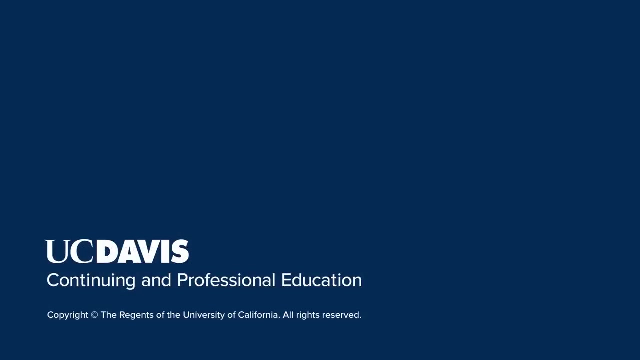 Okay, great. So now that we're here, we need to validate our form and actually get the data from this thing. once we're sure our form is validating, fine, And we'll do that in the next video- Great In our previous video. 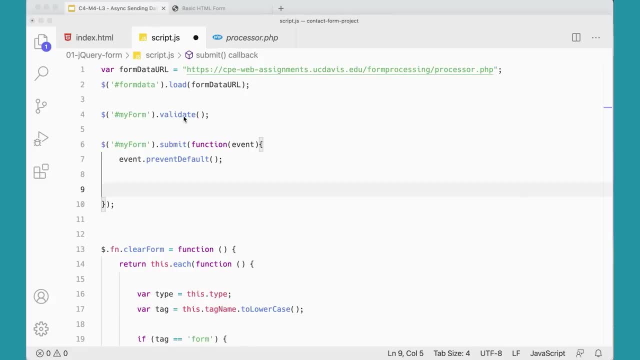 we started by validating our form and then capturing the submission of the form. Now we need to check if I'm going to put an if statement in here And I want to get valid this item here, my form, If this form valid. 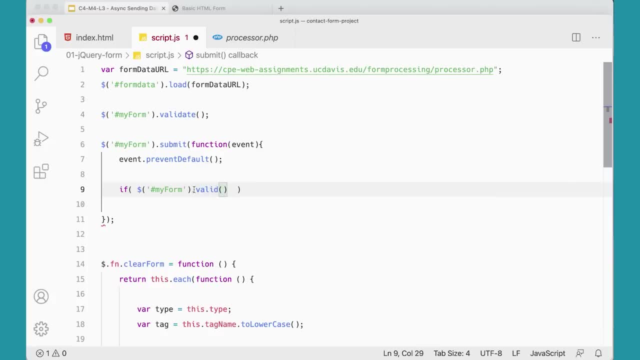 This is going to return true or false, And this valid function is available to us because we have the validator plugin added, So this is going to return true. So true or false, If it's valid or not. So if it's true. 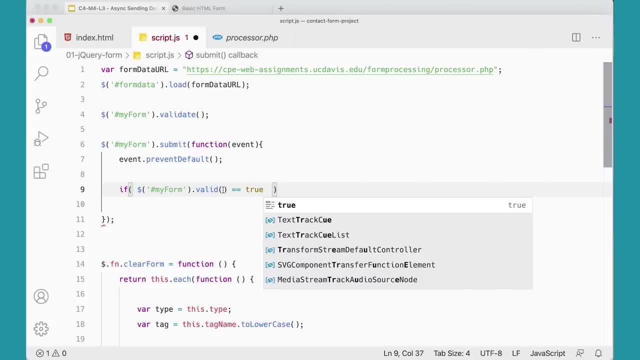 we're going to do something If this form is actually valid, meaning the fields have been filled out properly. If that's true, then we're going to do something. And what are we going to do? We're going to do this. 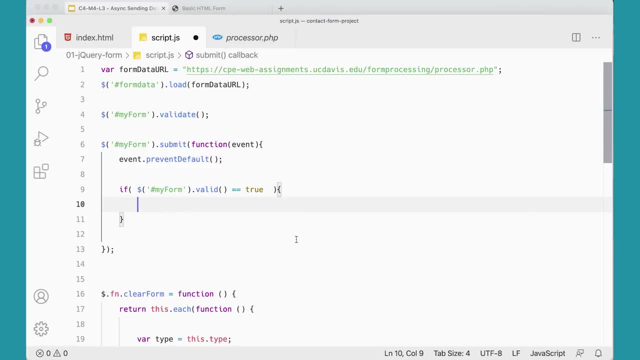 Oops, I had forgotten. I had copied that. We're going to do this. I'm going to make a variable called data string, which is really this form serialized, And so that's going to take the data string, and so that's going to take the data from the form. 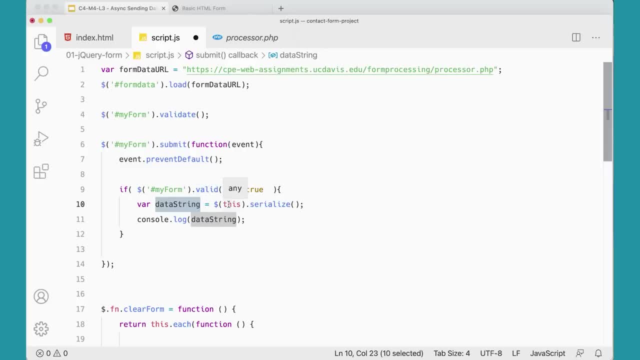 that we know is good now, because we've checked to make sure that it's good. So we're going to take it and we're going to serialize it And for right now I'm just going to console log out data string, just so you can see what we're getting. 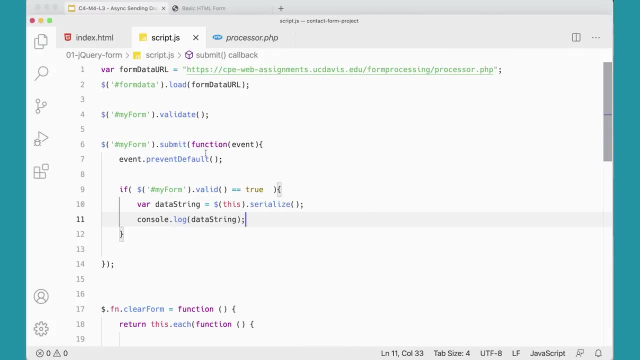 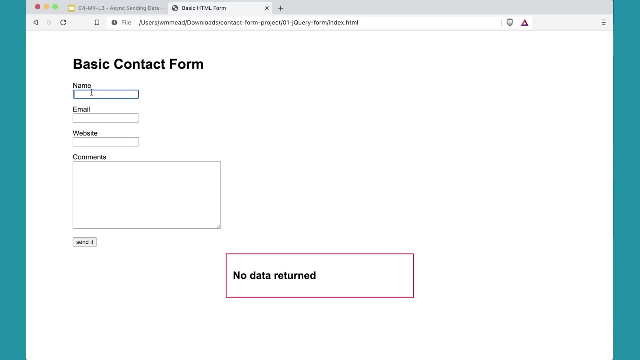 when we do this. So I'm going to save that and then come back to my script over here, My page over here, And I'm going to fill it out: Joe, Joe at somewhere. Joe dot com. Leave the website for now. 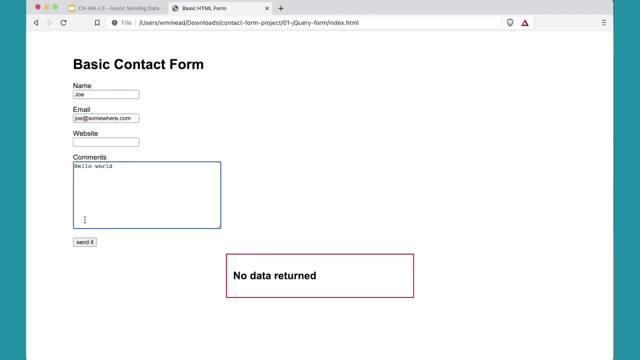 Hello world And I'm going to show my inspector and my console here And when I click send it you can see: name equals Joe. So that's the first field. Ampersand is my second field. Email equals Joe. Notice the at sign has been replaced by a percent 40.. 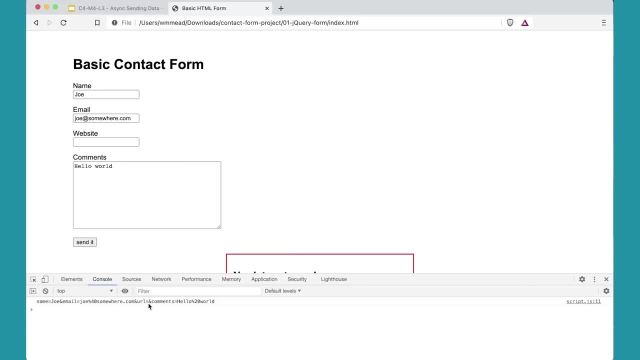 That's somewhere. Joe dot com. URL equals The URL is empty, so it's just equals, So it's empty. And comments equals hello, percent 20.. So it's put a percent 20 in where the space was, And so this data has been serialized. 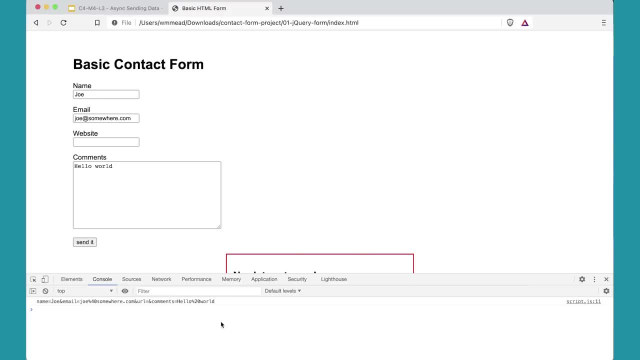 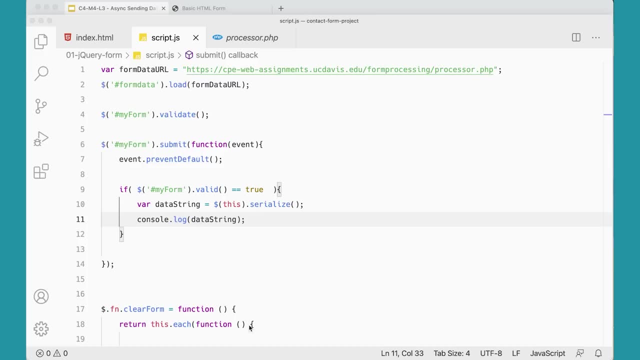 and turned into key value pairs, And some of the characters have been replaced so that it will be properly processed on the server. So that's pretty cool. Let's go back to our code and continue from here Now. at this point I don't need to console log that out. 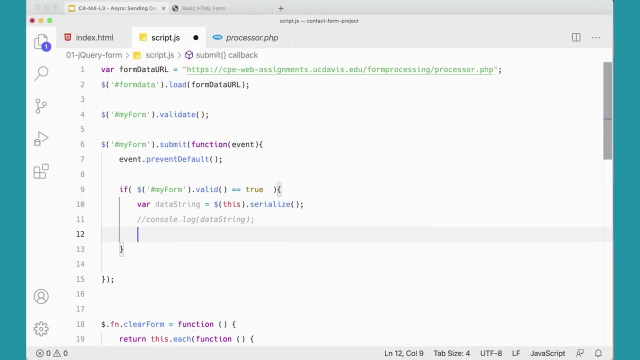 So I'm going to comment that out And I'm going to use my dollar sign dot Ajax jQuery method here. And if it looks kind of funny having the dollar sign period like this, just keep in mind that the dollar sign is short for jQuery. 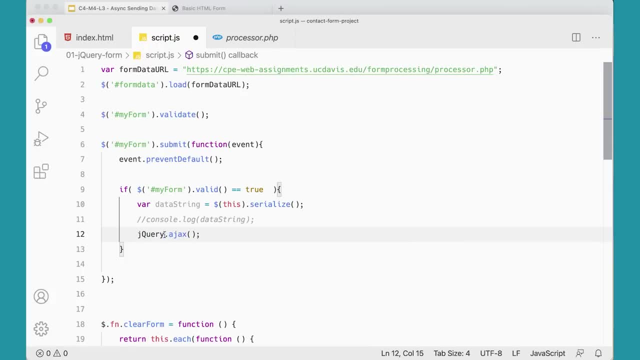 So it's really jQuery. So this is the Ajax method that is available to jQuery And that looks a little bit less weird. So it's really the Ajax method there. Dollar sign, Ajax, jQuery- the dollar sign is just a standard for jQuery. 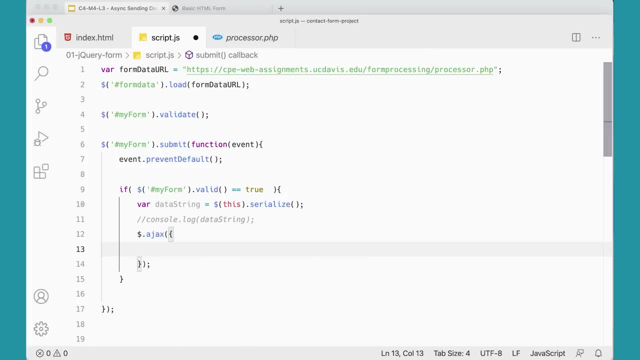 We're going to pass in an object here. I'm going to press return to make some room- And then we need to put a couple of key value pairs inside this object that we're going to need to send via Ajax. The first one we need is: 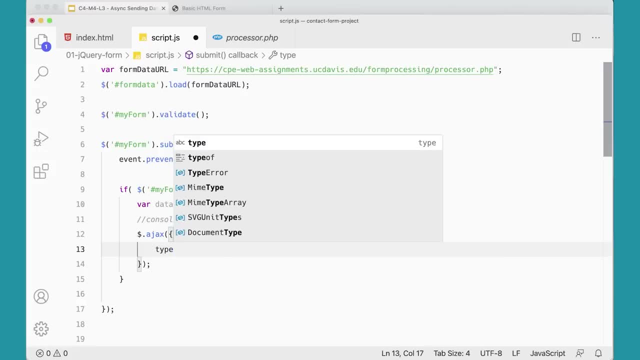 post type- Sorry type. And the value is post. You can send data generally by get or by post, And then we put a comma, because we use commas in objects to separate the key value, pairs and objects. The next one that we need is the URL. 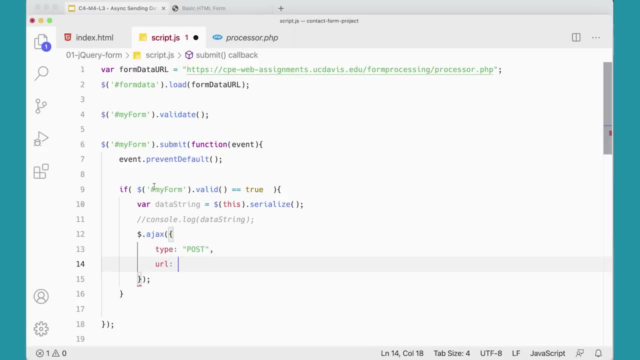 Where are we sending it to? Well, we're sending it to this thing: form data URL. We're sending it there. So we put that in And then we get a comma. What are we sending? What's the data that we're sending? 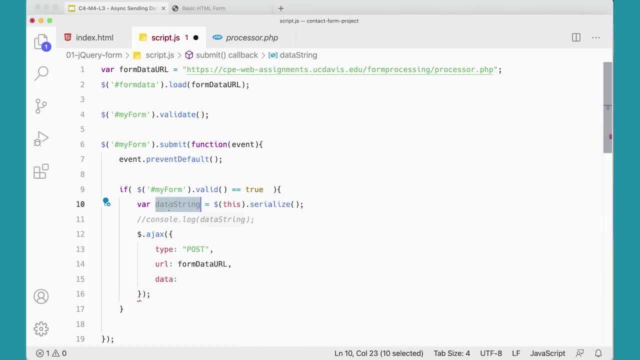 Well, we're sending this data data string- Great, So we get that. And then finally- assuming that it's successfully sent upon success, we're going to run a function like so, And the function is going to pass in the data. 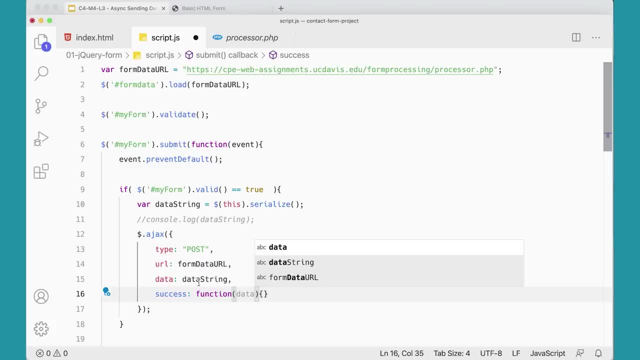 that it gets back from this data string. So we get the data back from our form And we're going to do a few things in this function. I'm going to move this curly brace down because I think it's a little bit easier to read. 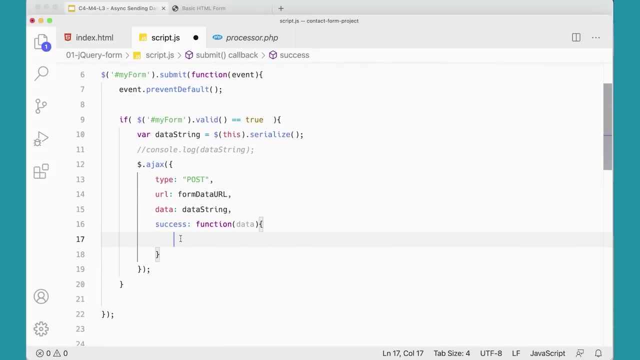 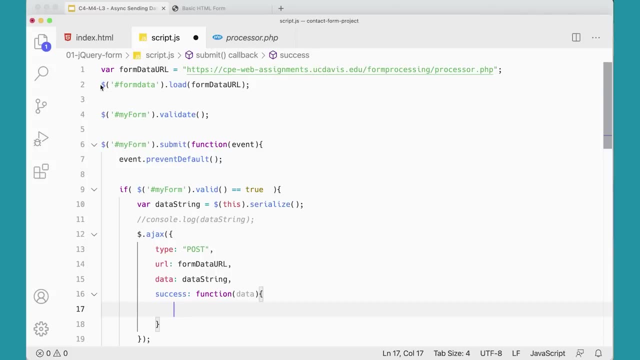 if we do it in two steps here. The first thing we're going to do is we're going to take this element, this form data element here, And we're going to do HTML and load data. So it's going to take the data that comes back. 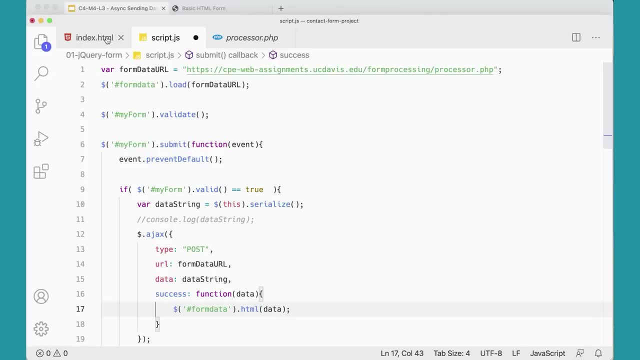 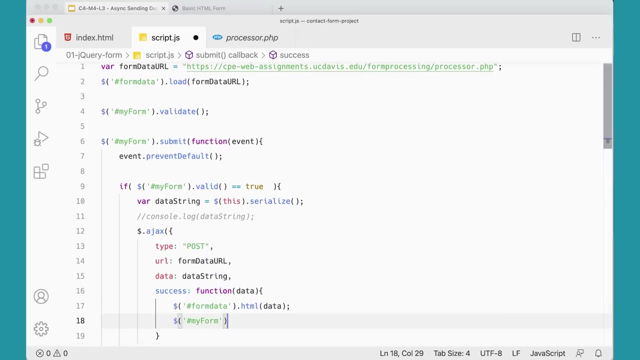 from a processor, PHP, and stick it over here in this HTML file, down here in this empty div. So it just puts it on the page, Nothing too fancy. And then we just want to take our form, this form here, and run this clear form function down here. 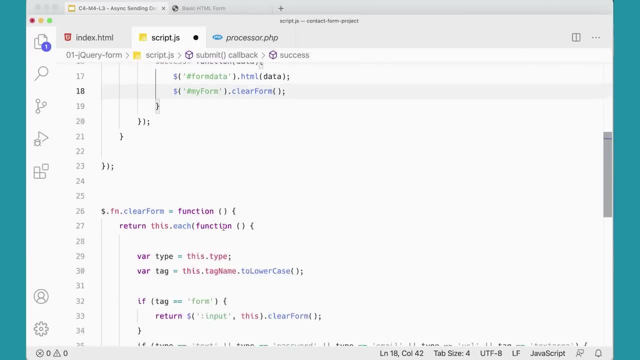 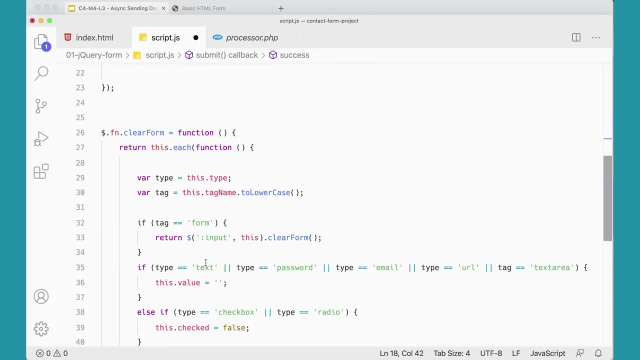 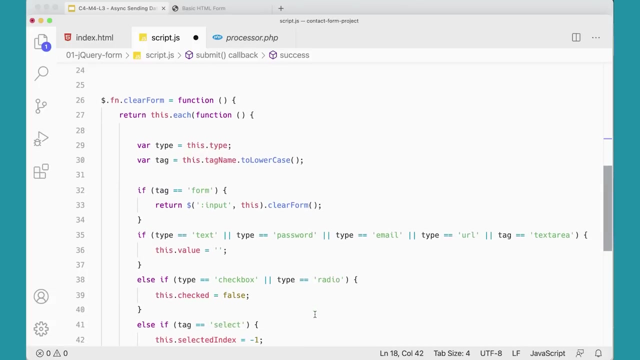 Clear form. If you come down and look at this function, all it's doing is going through and clearing out the, you know, setting the value for text fields, passwords, emails and URLs, and text areas to empty, If you had check boxes or radio buttons. 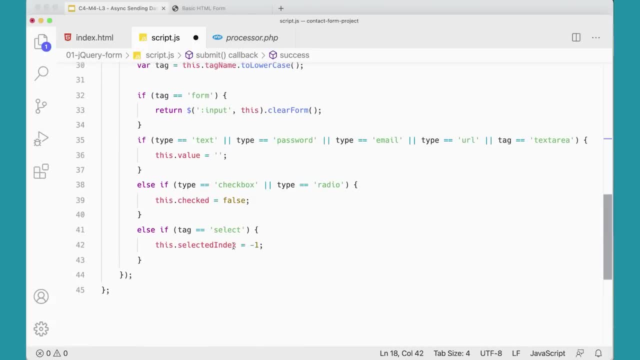 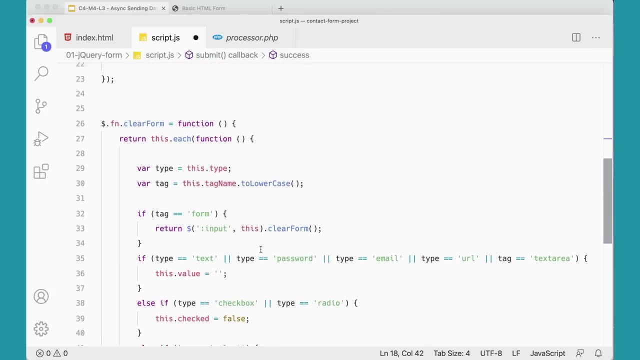 it's going to set them to false. If you had a select list, it's going to set the index to minus one. So it means nothing is selected. Everything gets emptied out. That's what this little function is doing down here. It's just clearing out the form. 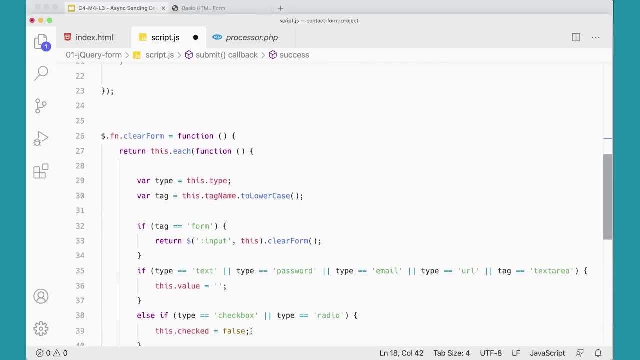 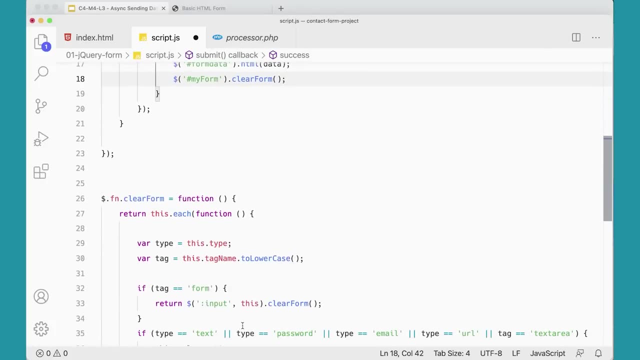 This is just a nice little generic jQuery function for clearing out any type of pretty much any type of form. You might come up with a few form fields that this doesn't clear out, but this will clear out most of them, So we're just clearing out the form there. 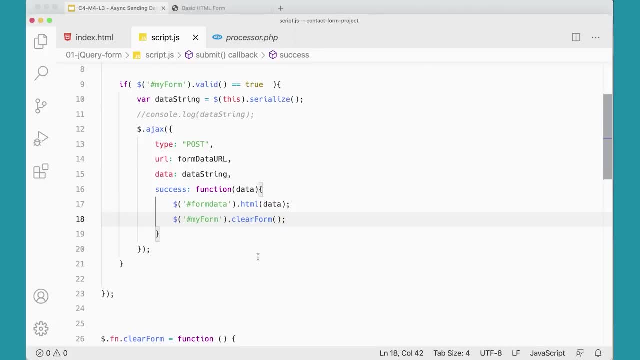 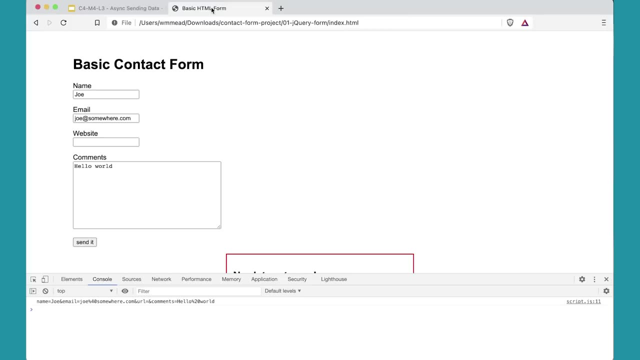 Okay, great, I'm going to save that and then let's test it. It should work. If I come back over here and I close my console log here, refresh the page. Joe, joe at somewhere, dot com. put in a llamas rule. 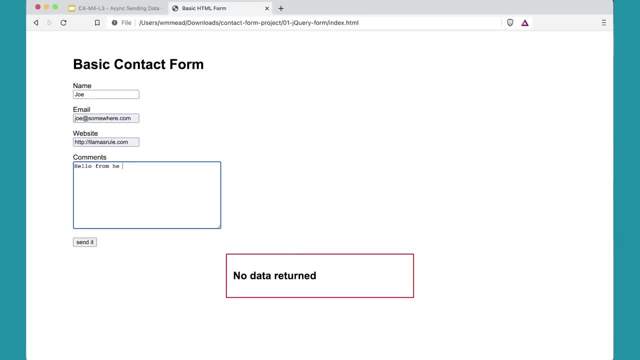 and hello from the llamas. And if I click send it and look at that it's going to that PHP file. PHP file is processing the data. then this page is loading that PHP file down here at the bottom of the page. 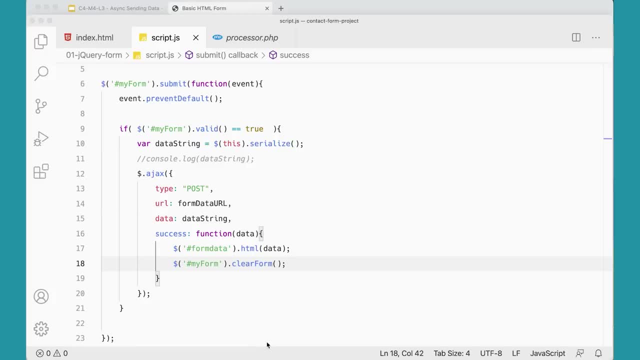 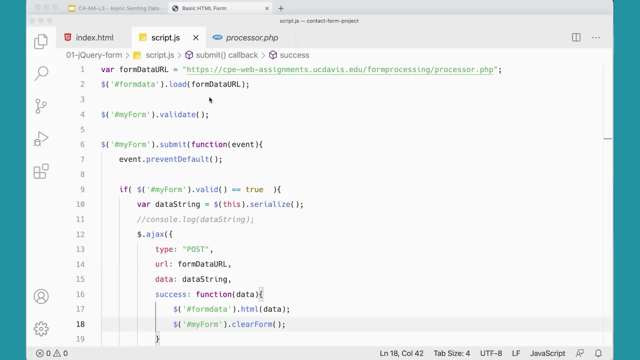 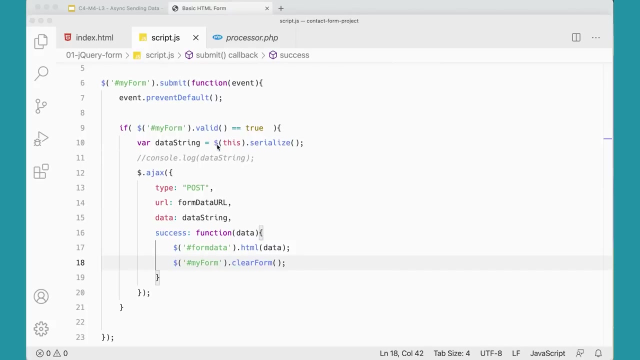 So that's working perfectly. So just to review here really quickly before we move on to the next part of this lesson: we're loading that page, We're validating the form And then, when the form is submitted, we make sure all the data is validated. 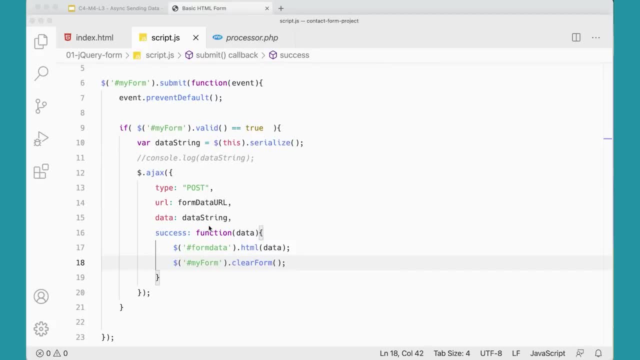 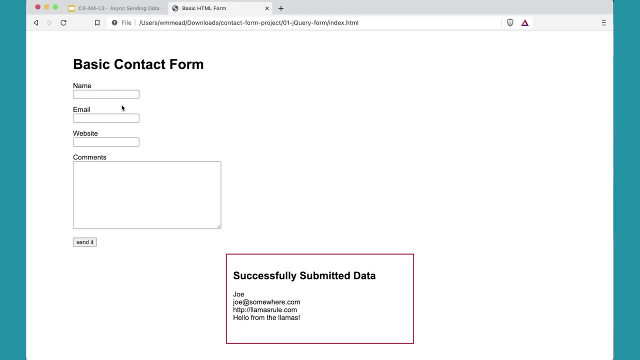 We serialize the data, then send it asynchronously to that PHP file, which then asynchronously gets loaded on our page. So this page never reloads. We're doing all of this stuff: We're filling it out, clicking send. It's getting the data and putting it on the page. 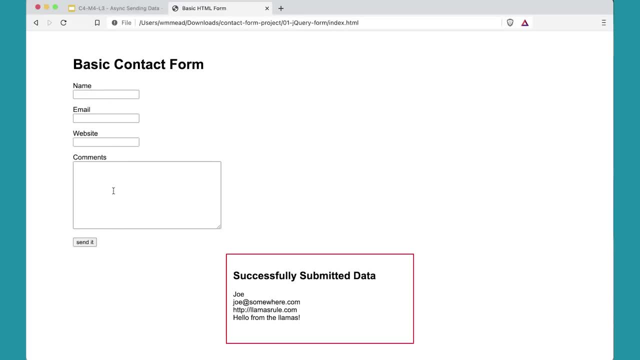 without ever reloading the page and then emptying out the form. We have to empty out the form manually because we never reload the page, So we want to empty out the form to put it back the way it was, in case we wanted to send some more data. 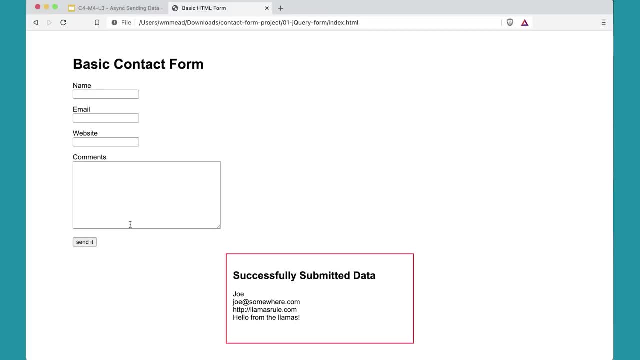 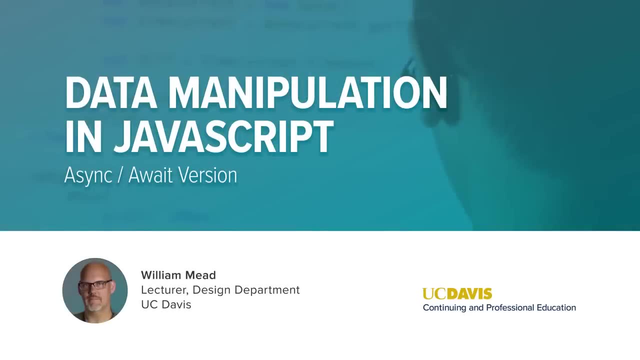 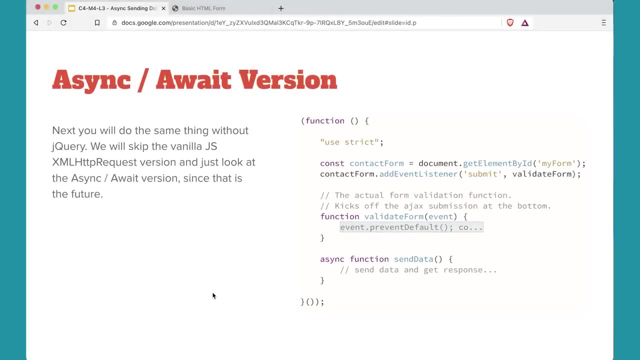 So that's all working really, really well And it's kind of interesting to see how you can do that kind of thing. We finished the jQuery version. Now we're going to do the version using async and await and VanillaJS. We're going to skip the VanillaJS version. 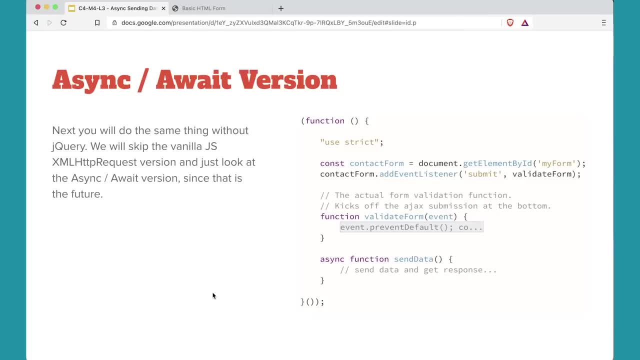 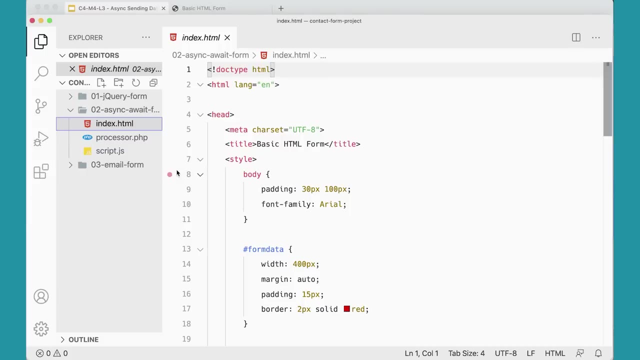 that uses the XML HTTP request version, and just look at this async await version, since that's really the future of where JavaScript is going Now. the JavaScript file. if you go look at it, the code that you need to do the validation is already here. 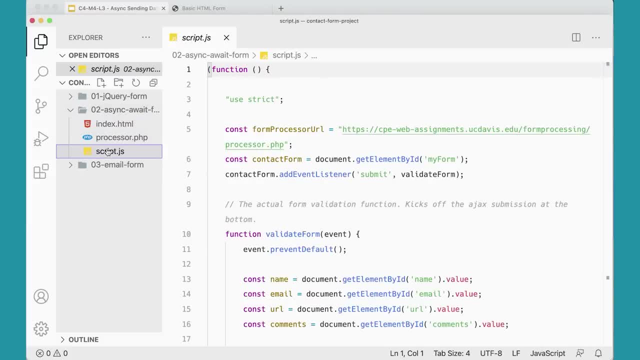 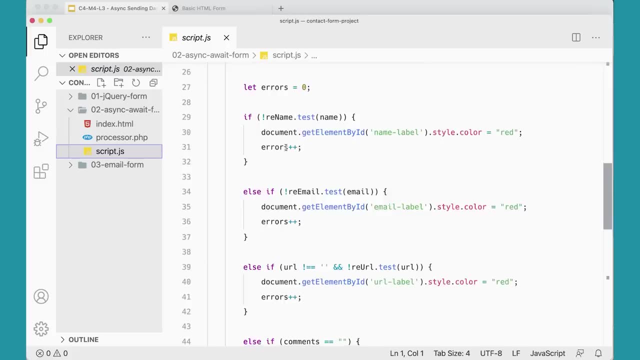 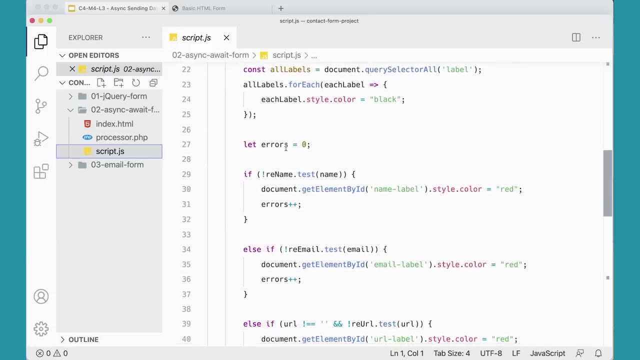 So here I am in my folder here And if you look at the script file, I already have the validation code in here. We did the validation work in a previous lesson And you should understand that this is basically just going through each field and testing it to make sure that it passes. 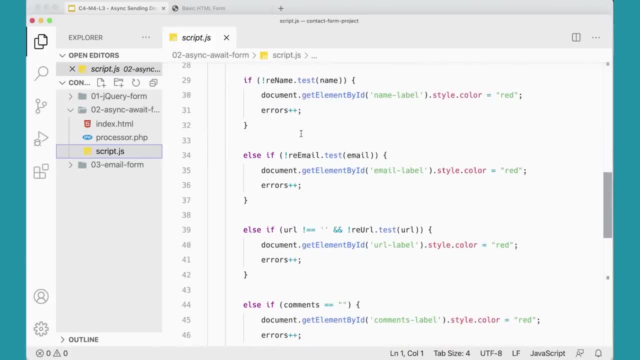 If it doesn't, then the errors variable gets incremented And down at the end. if it doesn't, if the errors variable is zero, meaning there hasn't been any errors and it hasn't been incremented, then we run the send data function. 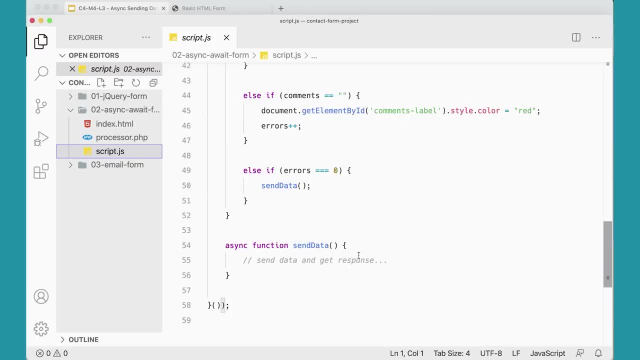 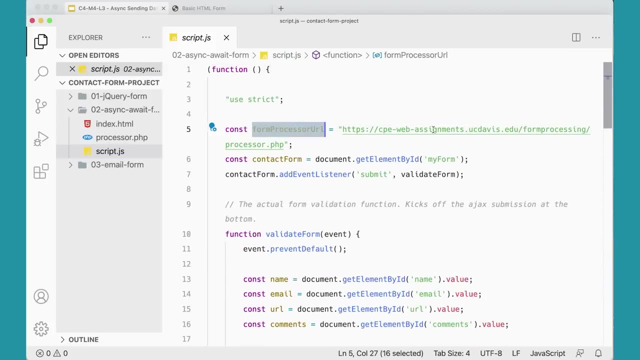 And that's what we're going to work on. We're going to work on just this piece down here and sending the data. You'll also notice, up here at the top of the page, I have a variable for form processor URL. that's that same PHP file that we were using in the previous version. 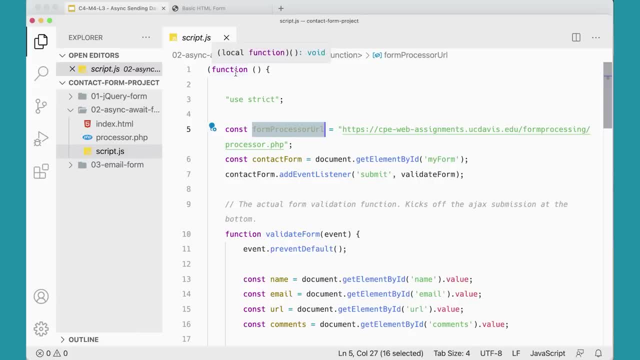 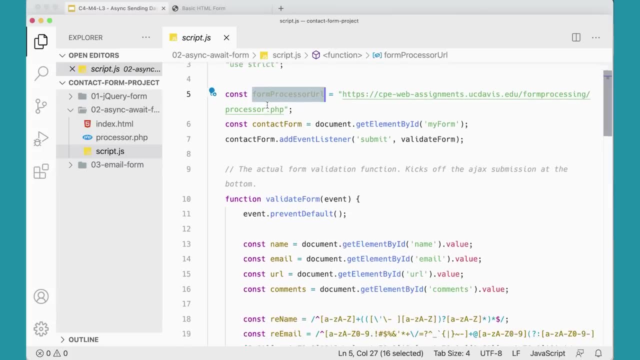 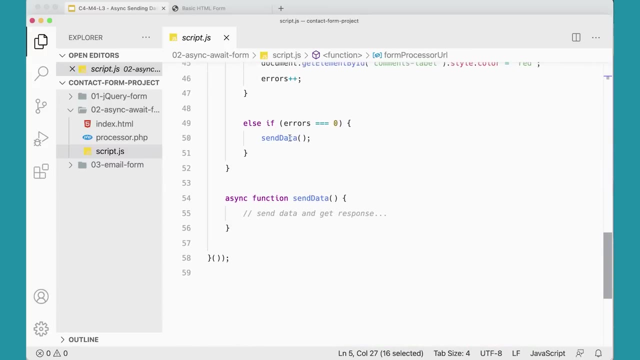 I have the whole thing inside an IIFE immediately invoked function expression For best practices with our use strict directive. So we're using all of our best practices in this and getting this ready to go. So if there are no errors, we send the data. 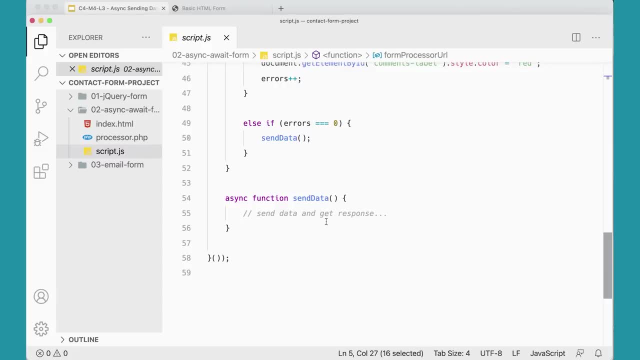 And that's how we're going to make this one work. So let's start to fill out this asynchronous function. We've got the async keyword here, So I'm going to get rid of this comment. I don't really need that And I'm going to paste in here. 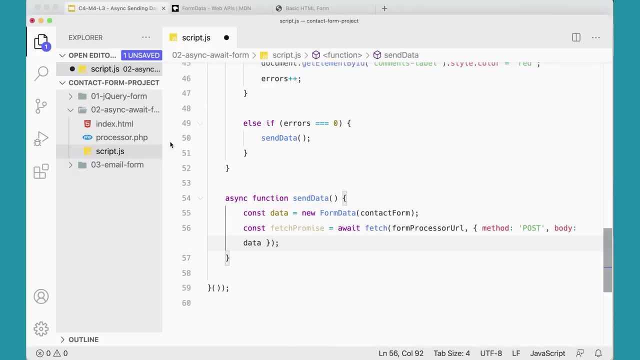 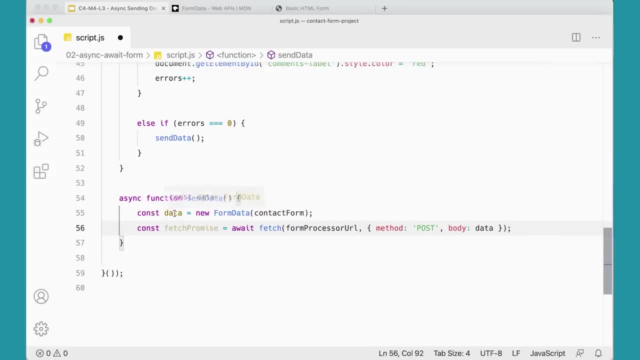 You're going to have to type this, but I'm going to paste it in here. I'm going to sort of close this explorer So this fits all in one line here, But I have a variable data that's going to go and get this. 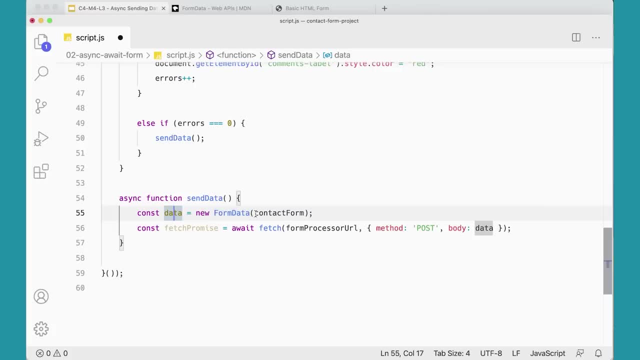 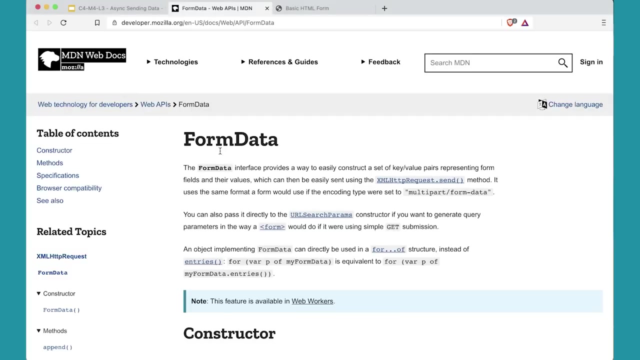 use a new form data object with contact form. This takes a minute to explain, but it's really kind of important here. The form data API- you can see it over here on the MDN website- does a similar thing that the serialize method does. 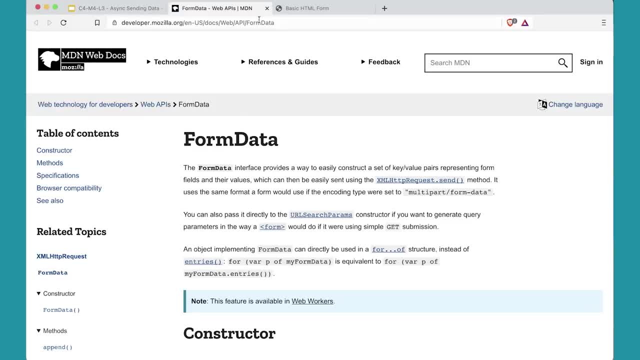 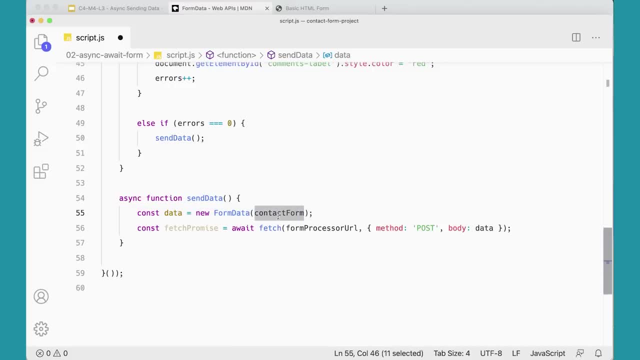 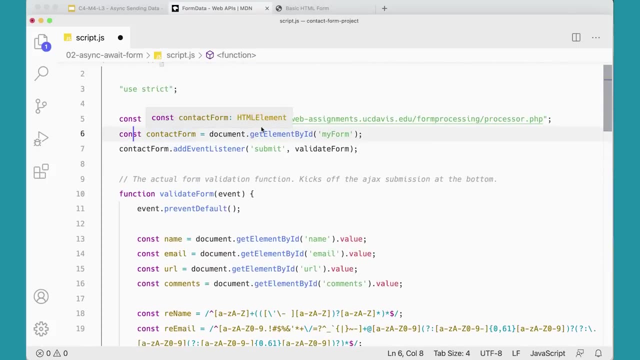 that we used in jQuery. So here we're using form data, which is going to get the actual form data from contact form, And contact form again is defined up here at the top of the page. here Const: contact form document- get element by a dmy form. 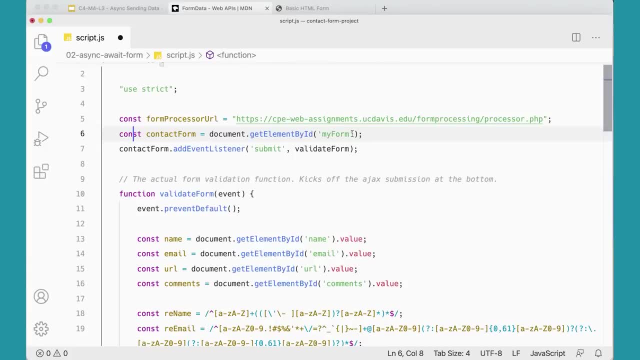 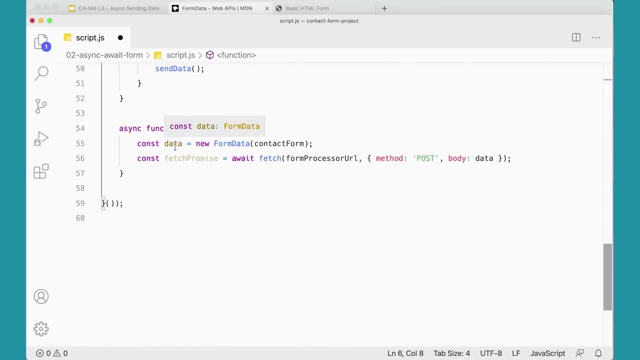 So that's just getting the form and taking the data from that form and sticking it and using this form data API to serialize it and stick it inside of data. Okay, And we know that that form data is good because it's already passed the validation. 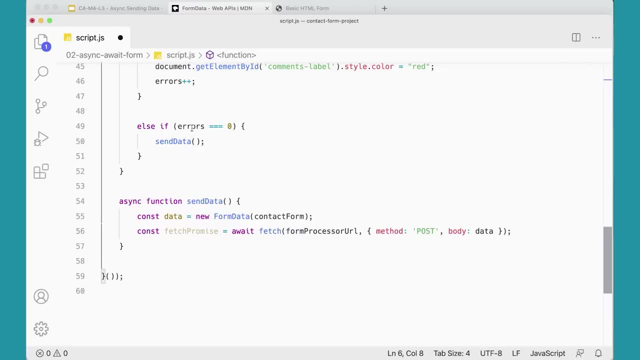 before the send data function even runs. So this function only runs if there are zero errors. Okay, So we know that is fine. Okay, So then we're going to make a variable fetch promise and we're using await with our async. Again, remember, these two things work together. 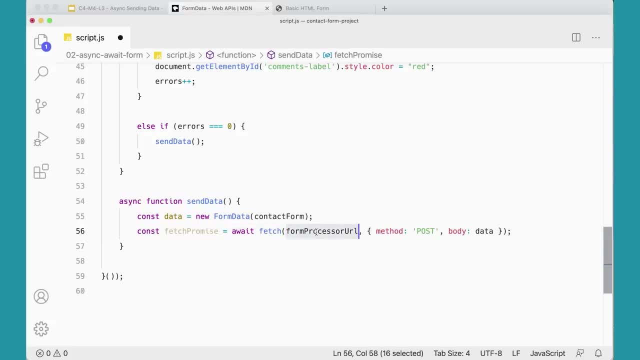 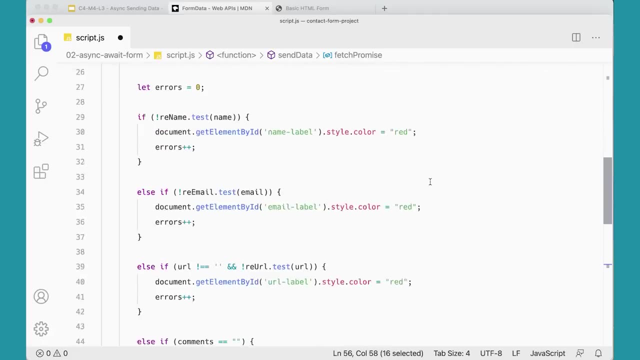 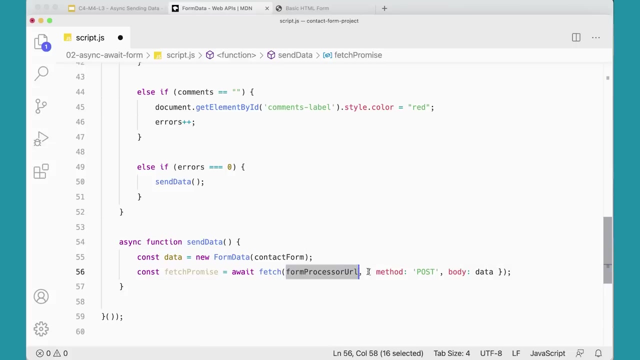 to use our fetch API to go to our form processor URL, which again is up here. That's this URL. You're going to just put this whole URL in there, but I have a variable to keep it a little bit shorter, So we're going to go get that form processor URL. 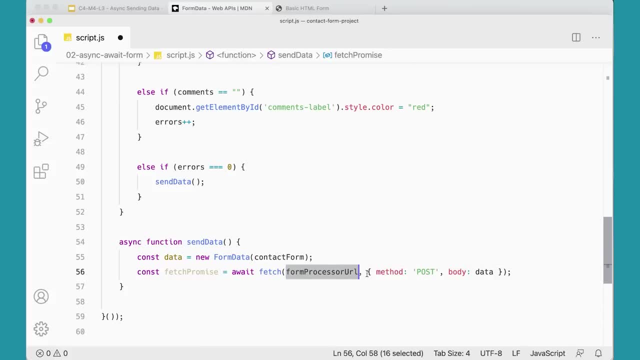 And this is the new thing- I've added an additional method here. This is a. we didn't see this before. Before, when we did our asynchronous exercises, we used fetch by just giving it a URL, but we didn't give it a second parameter. 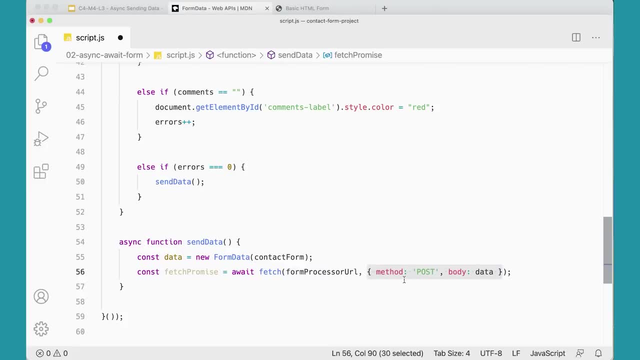 And the second parameter is an object that's going to send the data to this URL, And we're sending it by post. What are we sending? We're sending the body. We're sending data in the body. What's data? It's this thing here. 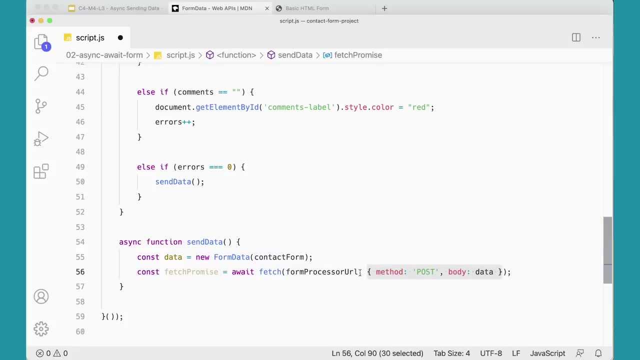 It's the data that we got from the form, So we're going to send that to our form processor, which is then going to process that run and process that form and give us back what it actually processed And that's going to be sitting inside of fetch promise. 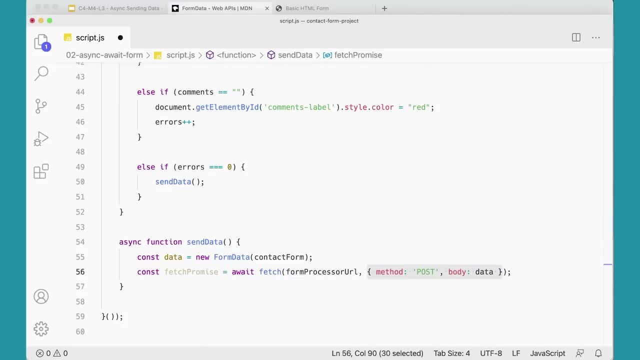 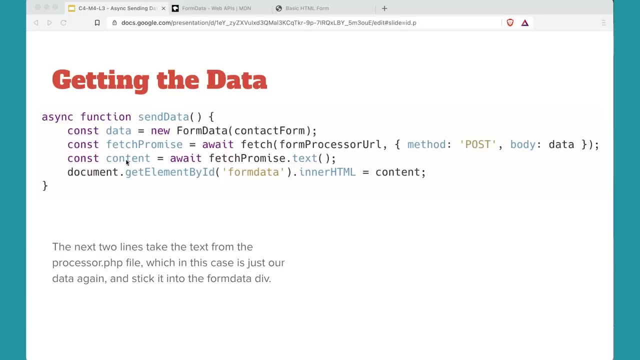 as you'll see in just a minute. The next two lines just get the text from that fetch promise text, because we're just getting some text from that processor file. We get that text using our await keyword, put it into this variable content and then add it to the page. 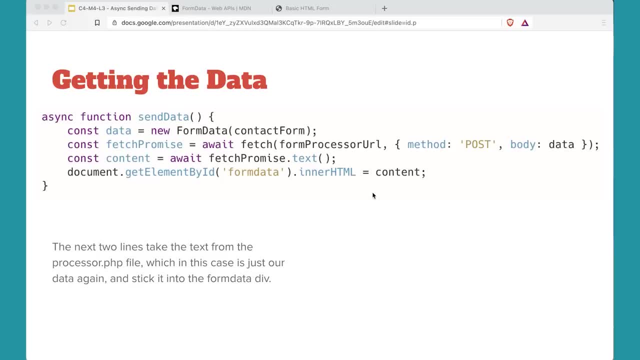 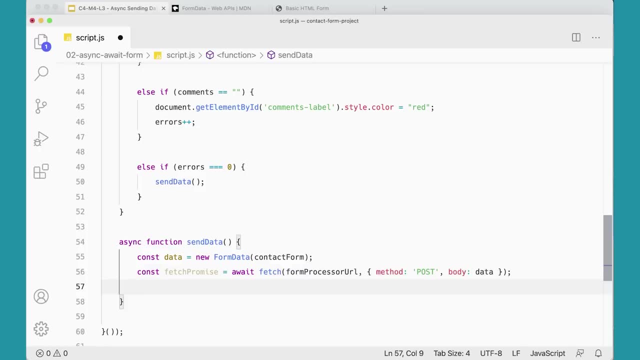 We're changing that inner HTML to whatever that content is, So that's pretty easy. Let's go ahead and add that in over here And you'll have to type this out, but I'm pasting it in too, so you don't have to watch me type it. 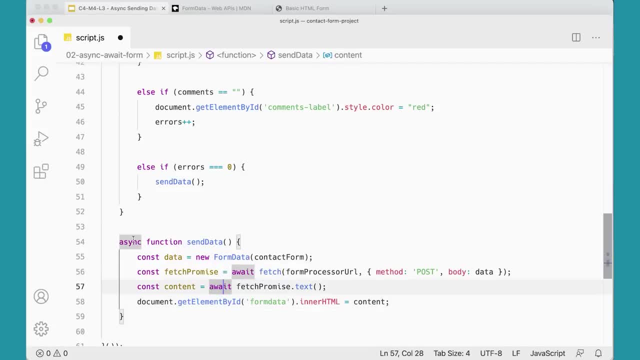 But basically, yeah, we're just going to use our await. Again, we're using await because we're doing this asynchronously with our fetch promise getting the text. And again, we're using text here because this particular file is returning text to us. 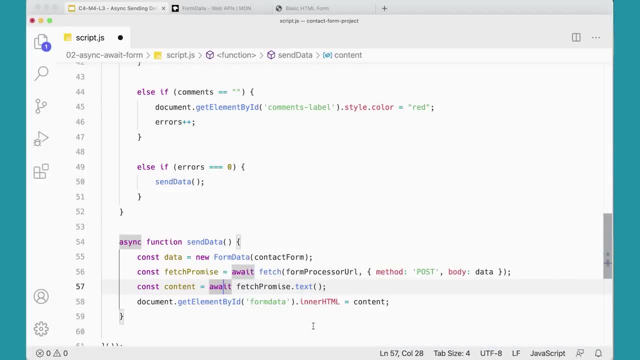 There's HTML in there, but HTML is basically text. We'll do something different when it's JSON information, which we'll look at in a little bit, But for right now we're just getting that and then putting it on the page. 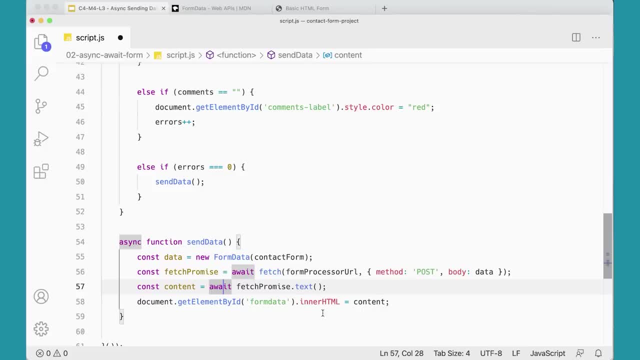 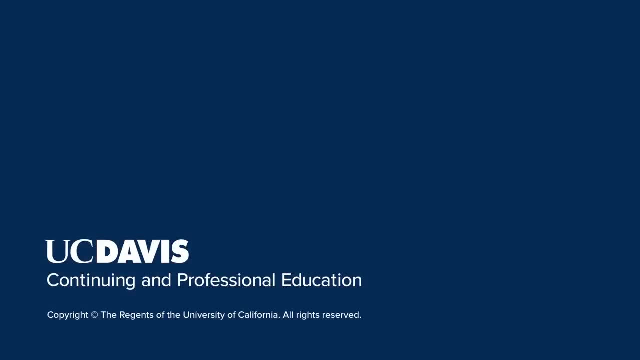 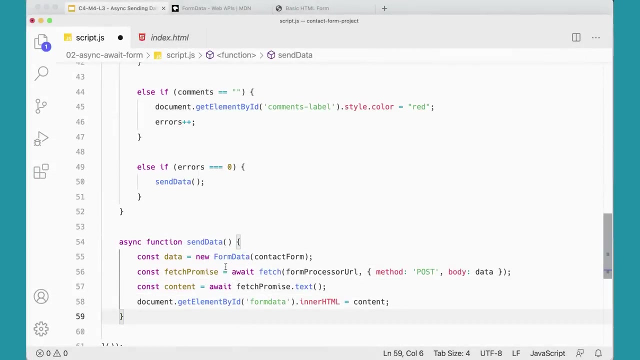 and that's all there is to it. We have one more thing that we need to do to this, and we'll do that in the next video. The send data function is almost done. We have it where we're getting the data from the form. 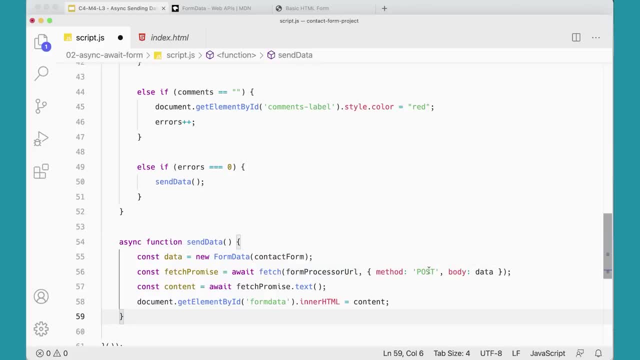 we're sending it to the form processor, sending that data there, getting some data back from the form processor, pulling the text out of what we got back and then putting that text on the page- The last thing that we really need to do- 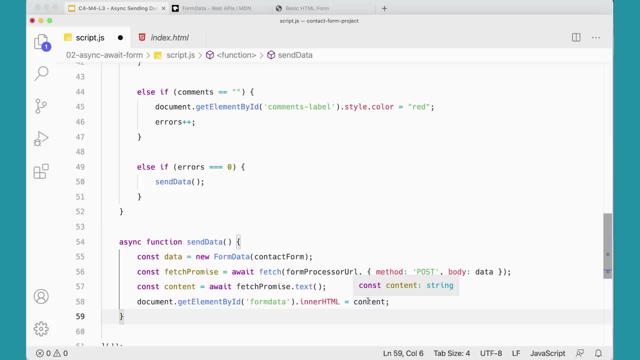 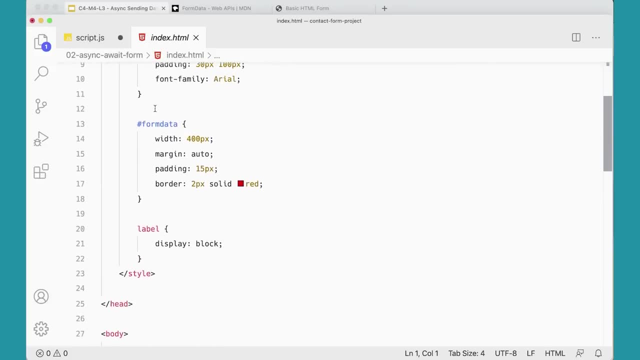 is to clear out the form, And for this I just want to look quickly at this index file just for a minute here, because this file is very much the same as what we used in the previous lesson. It looks very much the same. The only thing that you'll notice that's different. 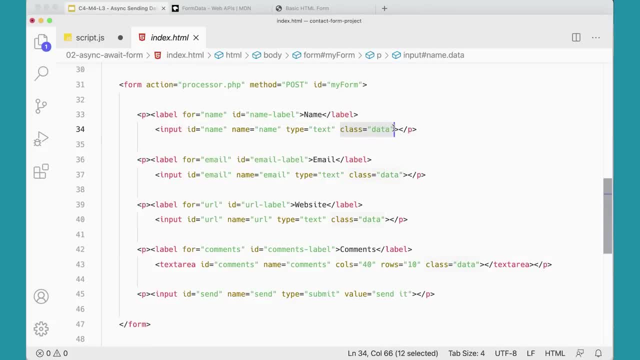 is. I've added this class data to these fields, the ones that we're going to want to clear out these three fields here. I've added a class data and we want to be able to clear that stuff out in just a minute here. 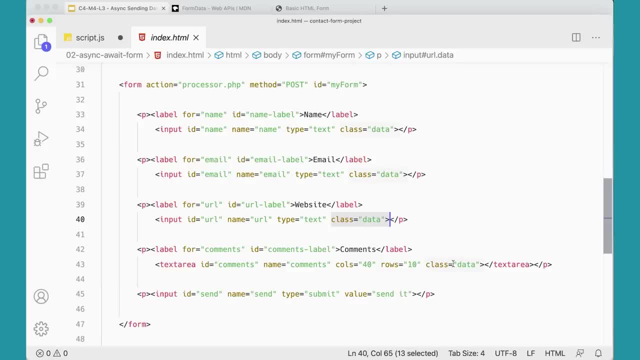 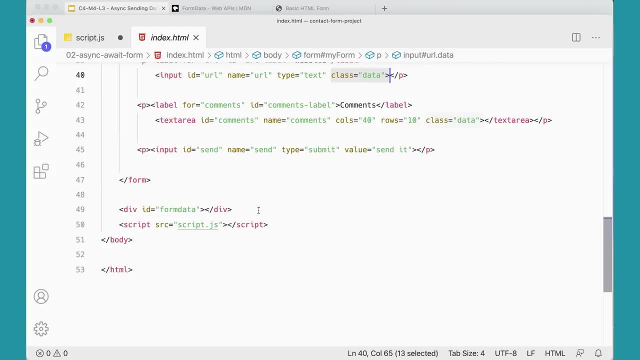 and this one down here too, So I've added that class data. The only other thing that's different about this is I'm not loading it. I'm loading the jQuery library and the validator plugin, which saves us some bytes of data to download. 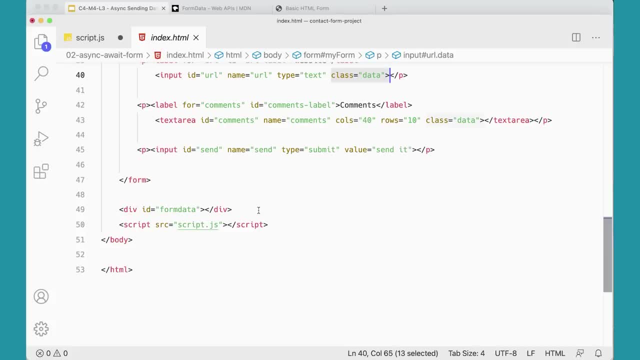 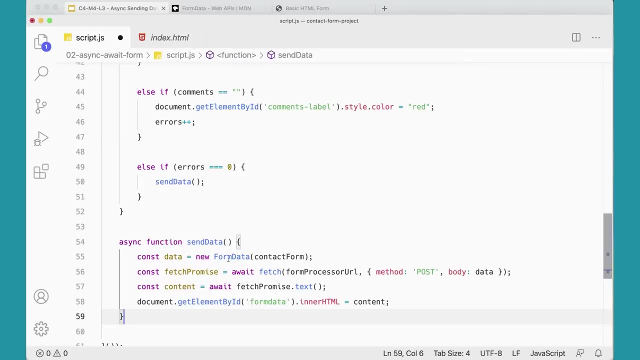 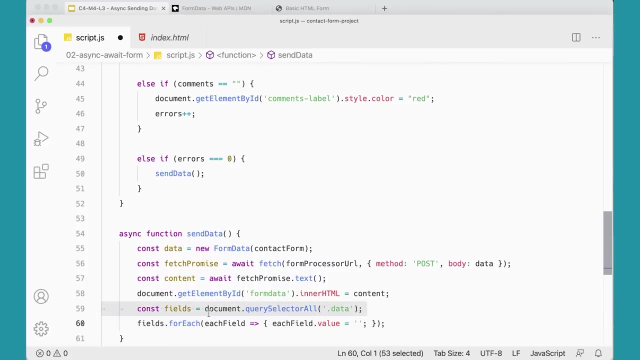 We don't need to download that whole jQuery library, just to do a little bit of validation, which is kind of nice. Let's go back to our script file and add these last two lines in here. The first one of these, line 59 here. 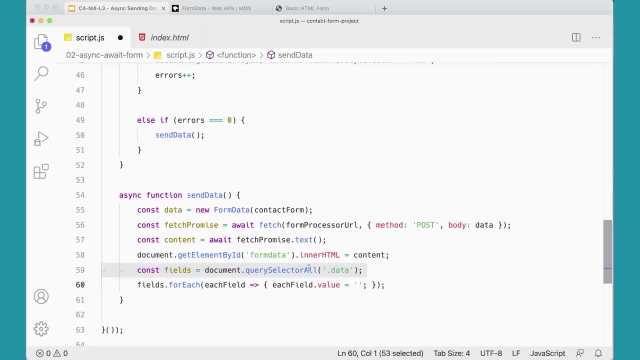 is just going to go in and get all of those fields that have the class data query selector, all So it's just going to go and gather all of these and put them in fields, which is now an array, And I need to loop through the array. 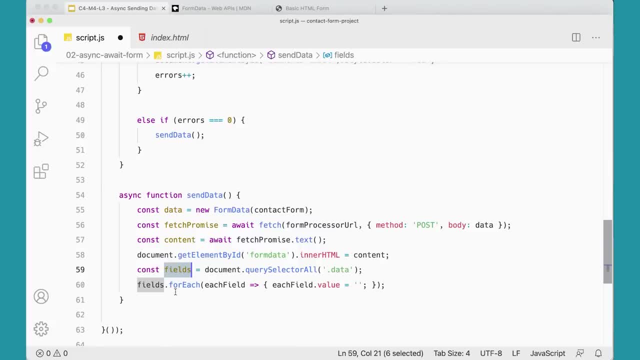 and clear out each field, And I'm doing that here in a nice little one-line shortcut, shorthand kind of way, using an arrow function which we've talked about in a previous lesson. We've talked about them quite a bit and hopefully you've had some practice. 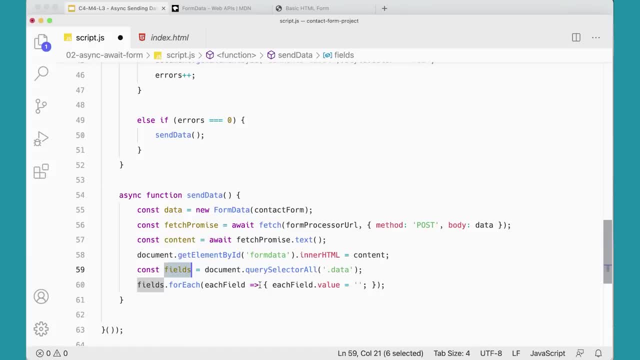 with arrow functions. now, If it looks weird, you can take the arrow function out and do it without it, but that's okay. But I'm using the forEach method on this array item and each field. it's going to loop through and get each field out of this array. 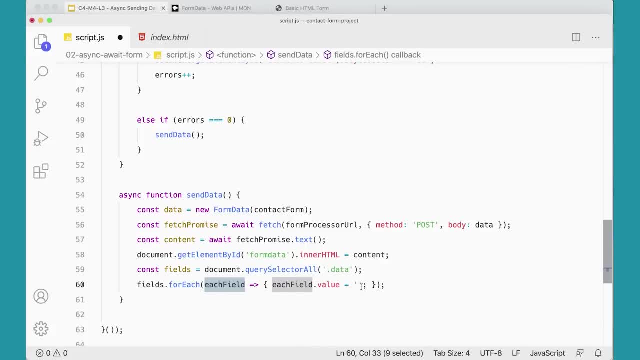 and set its value to empty. Now this is not nearly as sophisticated a form clearing out function as the one we had in the jQuery that we'd go through and clear out checkboxes and select lists and all that kind of stuff. This is kind of quick and dirty. 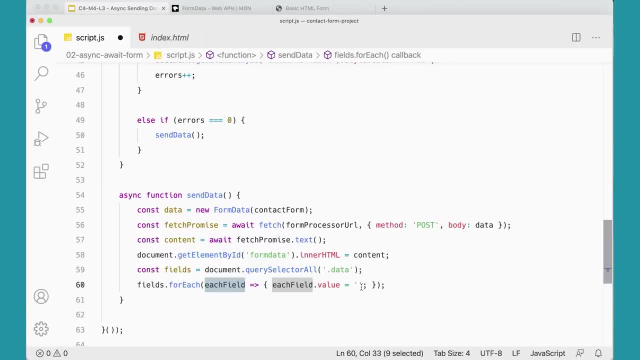 but for this particular form we don't need all that stuff anyway. so I figured this is kind of a nice shortcut way of doing it and it gives you a chance to kind of practice the skills you've done before. Try writing this in a couple different ways. 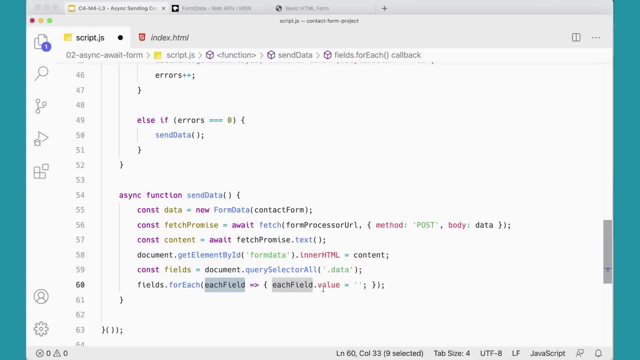 Try using it without the. see if you can get it to work without the arrow function. Or you could do a regular for loop or a for of loop, Because this is an array you can use for of to go through and clear them out. 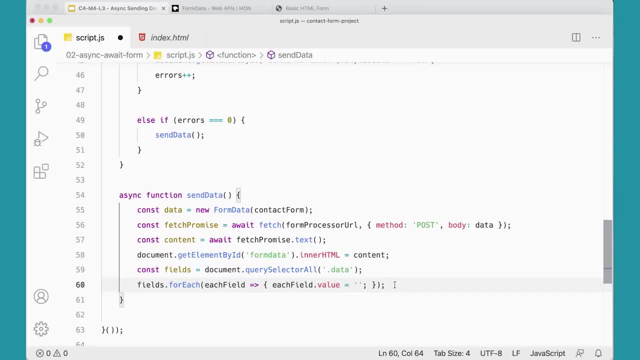 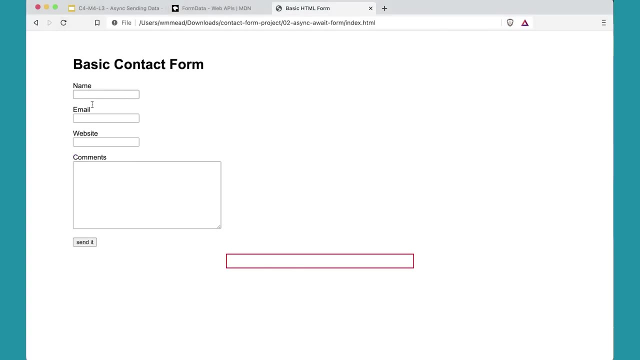 There's always lots of ways of doing things in JavaScript and this is a good example. But great, this should all be working now, so let's just test it. If we come over to our form over here and refresh this page. if I click, just send it. 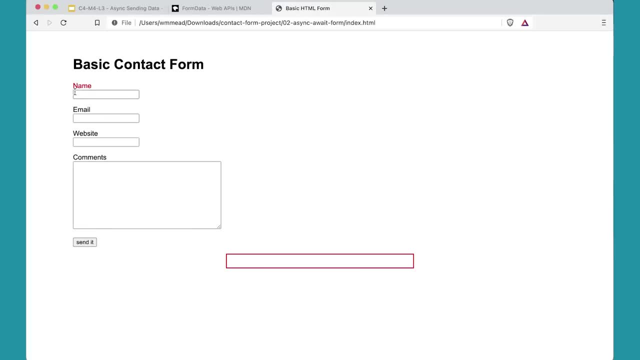 I should be getting my errors coming in here and that's working, So that's good. But if I fill it in, email, go to somewherecom website. llamas rule- hello world of llamas. Llamas are such funny looking creatures. 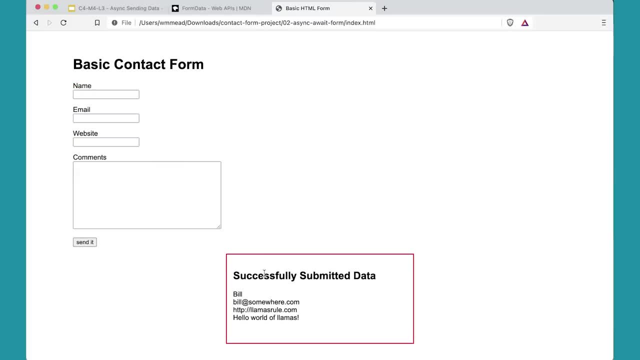 I always love them And look at that. it's working. So, without refreshing the page at all- we've not left this page or refreshed it at all. We've filled in the form, clicked the button. that click was registered. 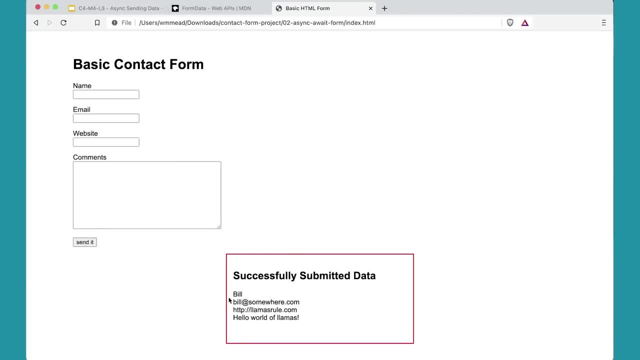 it validated the form and then came over and got the data from our file, sent the data to our file, the file processed the data, returned the data, which was then put on the page, and then the form was emptied out. So all of that happened without doing any kind of refreshing at all. 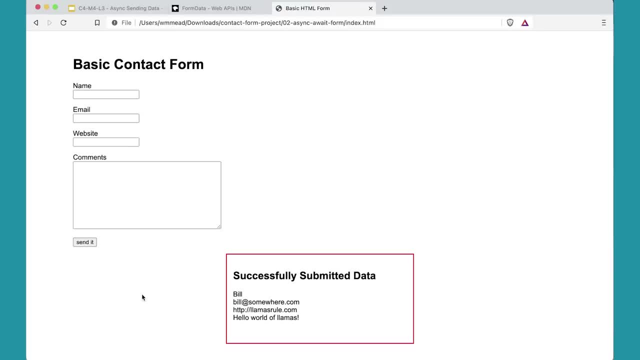 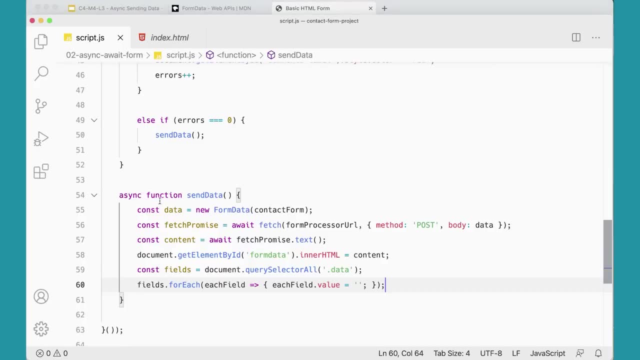 which is really pretty awesome and gives you a really good example of how this works, And hopefully this code here is looking familiar, because we did a lot of this in a previous exercise, And also I think it's worth pointing out that the difference between this and the jQuery version 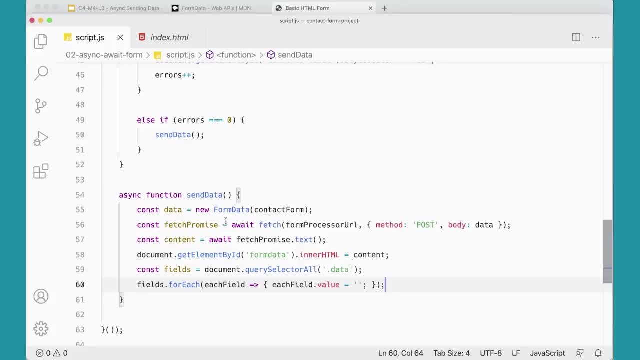 is really not very much. Both of them are doing the same thing. They're serializing the data, they're sending the data to the, the file, and then, if it is successfully returned, and if it successfully gets there and is returned, 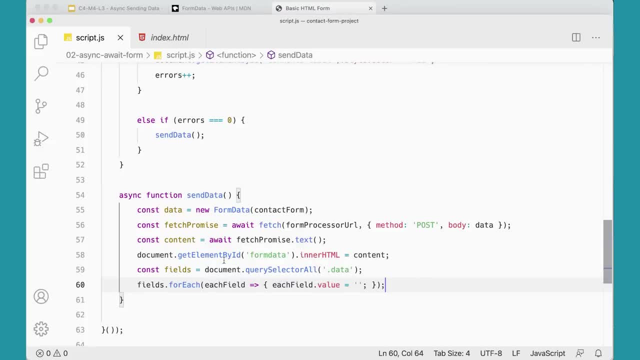 then we can process it and clear out our fields. All of these are being done Here with the async and await. it looks like it's happening just as a normal function, but it is actually. if it takes some time to actually reach the server and do this stuff. 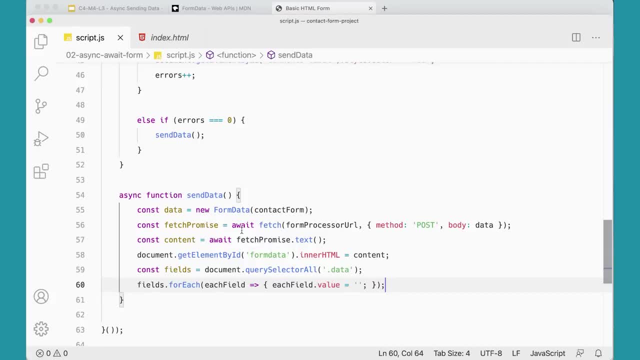 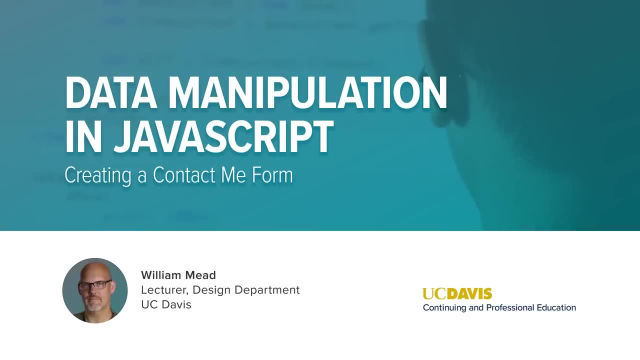 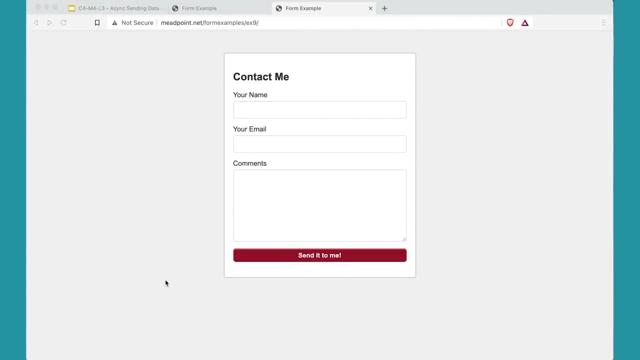 these things will wait until we get the data back, which is really pretty awesome. For the final part of this lesson, we're going to create this contact form here, And I'm looking at the finished version of what we're going to get. 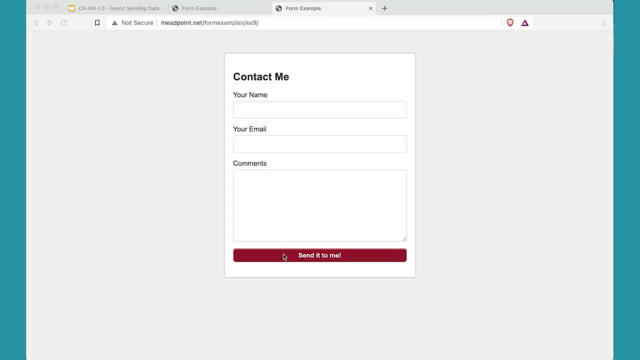 which if you try to send it and there are errors, you'll notice. if I click send to me here it comes up and says oops, and gives you an error message And then that fades away. And if you click send, 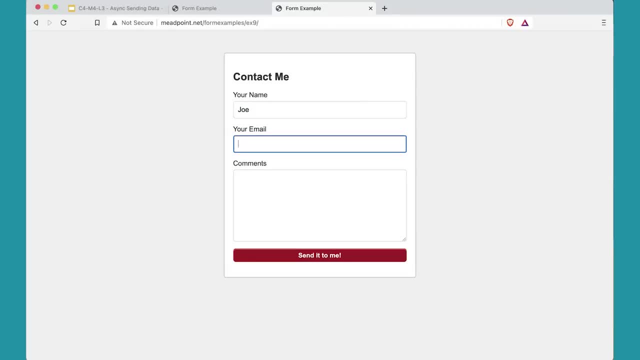 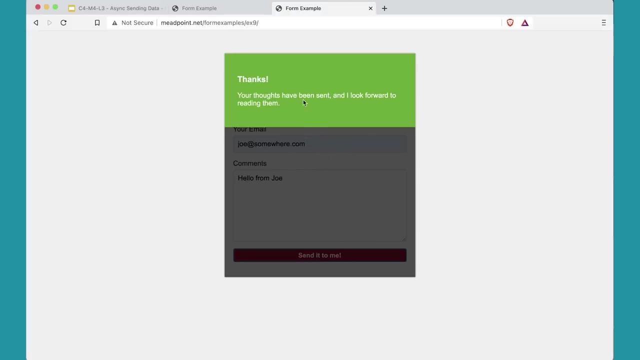 it puts the cursor into the field As you fill it out: joe at somewhere dot com. Hello from Joe, And then click send it to me. You get this nice little spinning effect and then you get a success message and then that goes away. 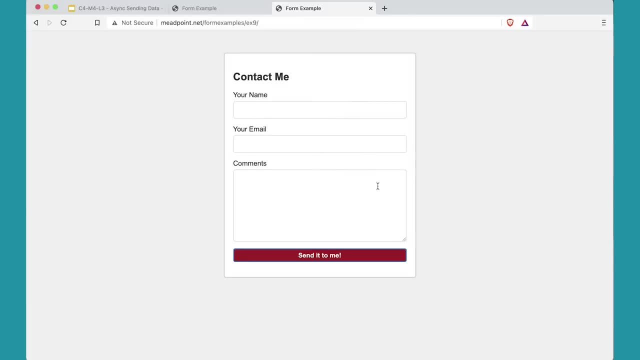 and then the form empties out. So it seems very simple and it is fairly simple, but there are a lot of pieces to this. We've got some nice interface elements happening here And in the end you'll have kind of a nice looking form that you could use on any website. 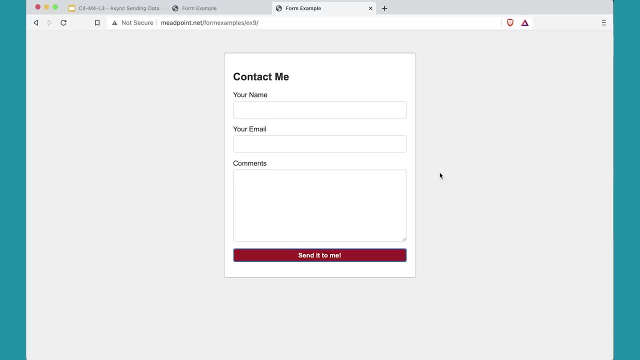 and actually send email, So that's pretty cool. So that's the working version that we're heading towards. Let's take a look at our files really quickly here. If we come back to our project here, I'm now working with O3,. 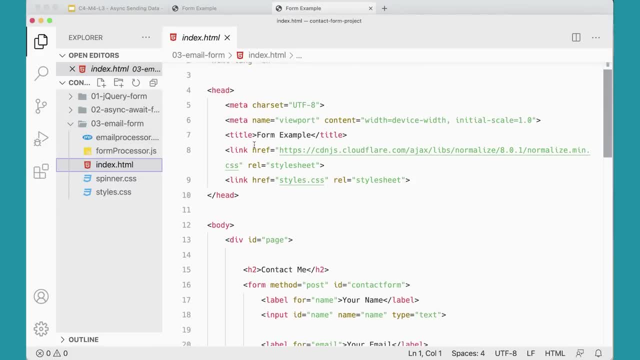 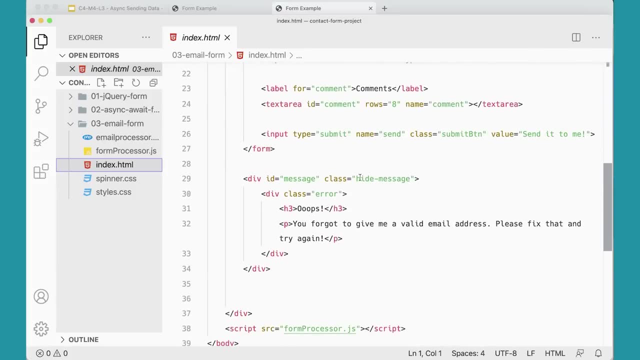 the email form files and the index files here and you can scroll through and see what's on here. but it's just a very simple file. You'll notice down here I have a message that has a class of hide message with a div with an error in it. 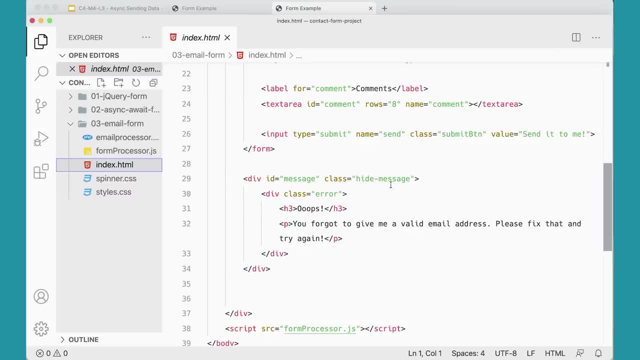 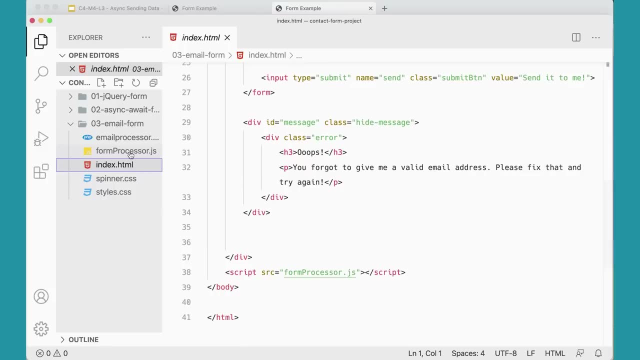 And currently, if you look at the CSS, hide message means set to display none, So this is not showing on the page. And then down here I'm linked to my form processor JS. This could be just scriptjs, but I called it form processor JS. 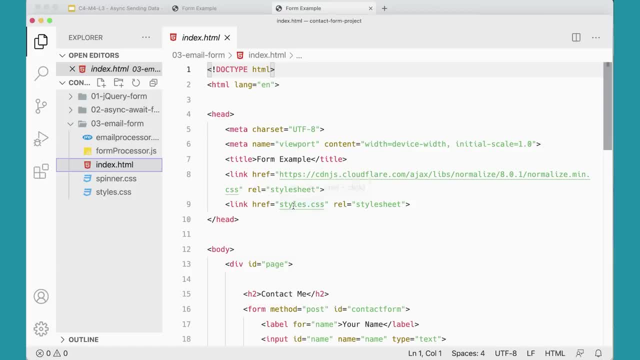 Okay, So there's there, There's that, And I have a style sheet linked and I'm linking to the normal file And then I'm linking to my script and all that kind of fun stuff. The spinner is a CSS thing. 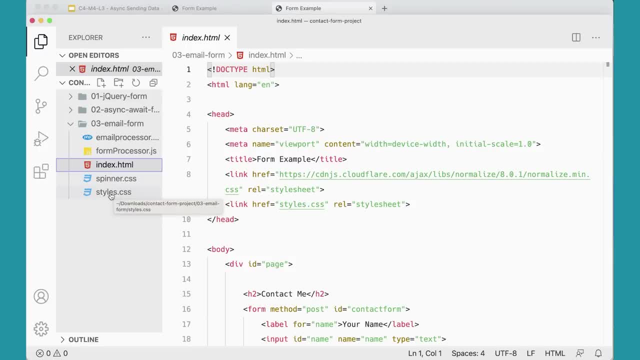 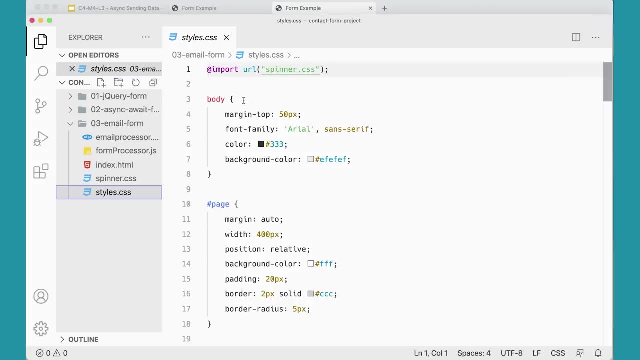 That's what's creating that little spinning thing there. You can look through the CSS file if you want to. That's kind of cool. Notice, this is importing the spinner CSS. That's where that's coming from. I didn't write that spinner CSS. 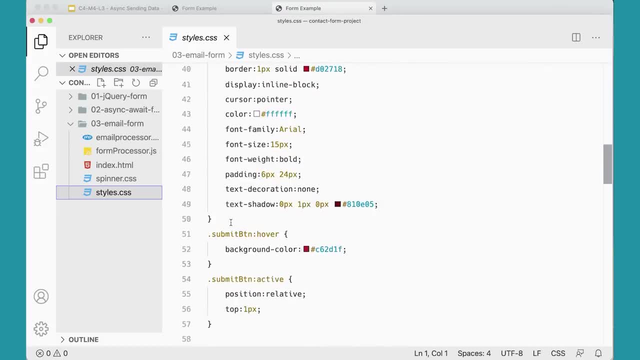 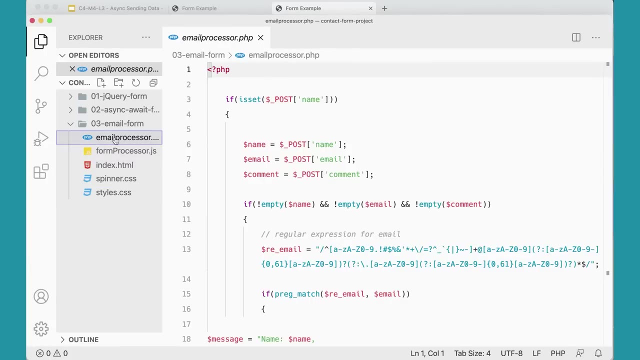 I downloaded it from somewhere so long ago now I don't even remember where, but I've used it off and on over the years, which is pretty cool. Also, we have our form processor, our email processor file here, And this is worth taking a look at just for a minute. 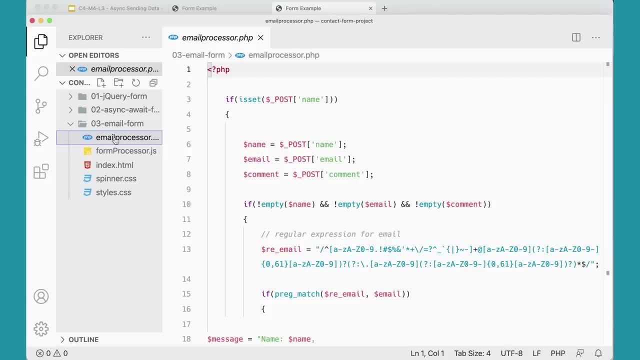 just because it's a little bit different than the other ones And, again, we're going to access this on the server. I'm putting it in this folder just for your reference, but you could actually use this file in your own server if you wanted to use this as an email form. 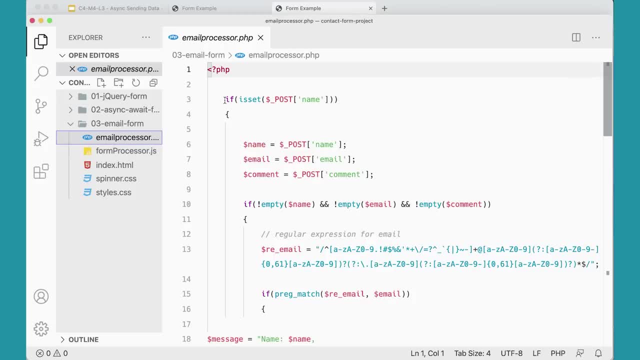 for your own projects. And what it's doing is it's just checking to make sure that the data was sent, putting it in some local variables, making sure the fields are not empty. Again, we're doing some server side validation just to make sure that for our own safety. 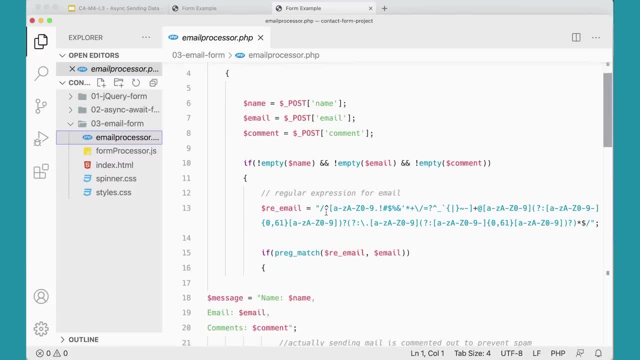 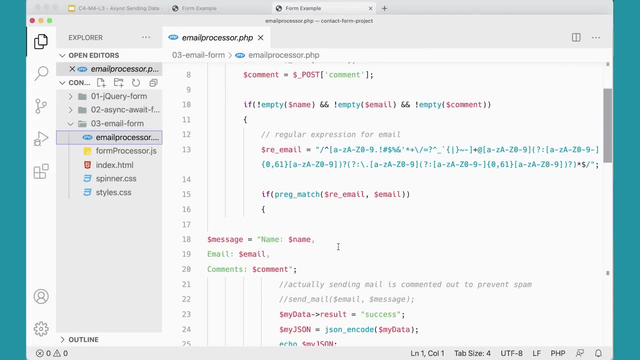 that people aren't putting bad things through over here. I've got a regular expression to check the email against to make sure that the email actually matches the regular expression. Somebody didn't put something other than an email in there And then I'm taking 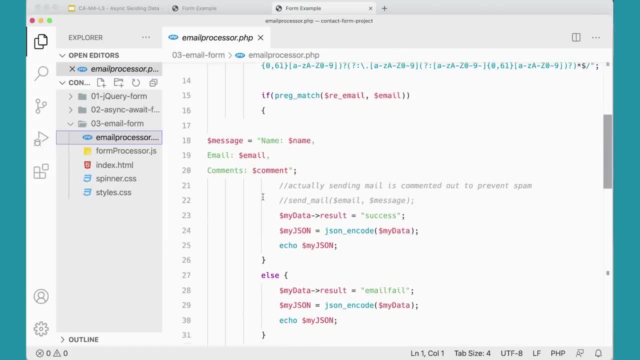 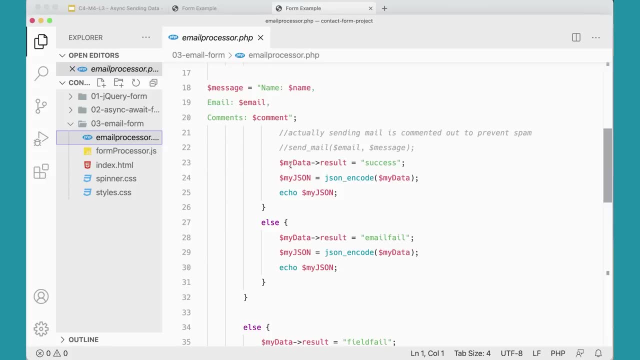 the message and the email and the comments and putting this stuff out here. You'll notice my data result success. This is actually creating an object called result And I'm encoding that and sending out some JSON that will say that will consist of one key value pair. 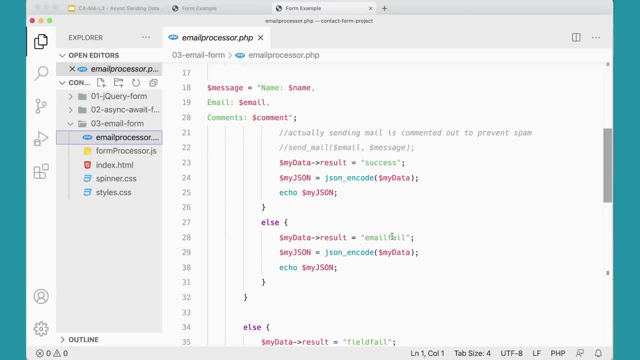 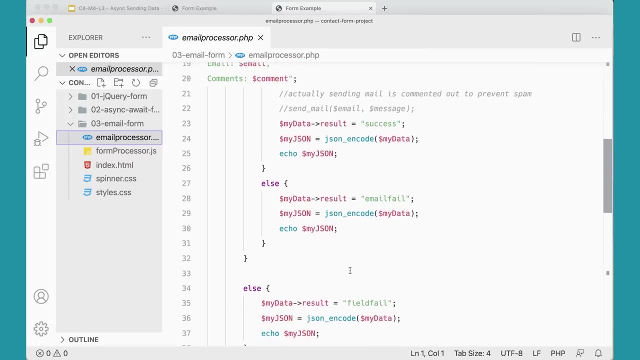 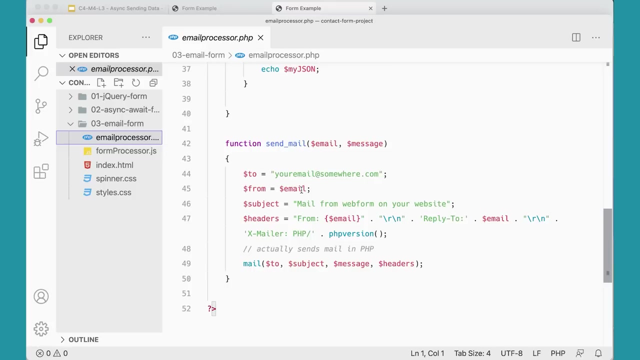 result, success or result and email fail. It's one or the other. If it doesn't work, then it'll send out something that says that it failed. Okay, Down here is the send mail function And this if you were to use this on your own server. 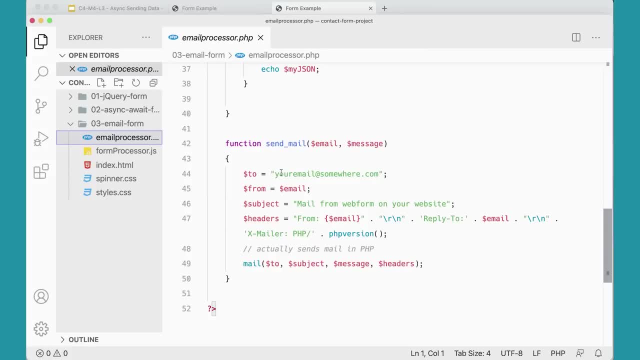 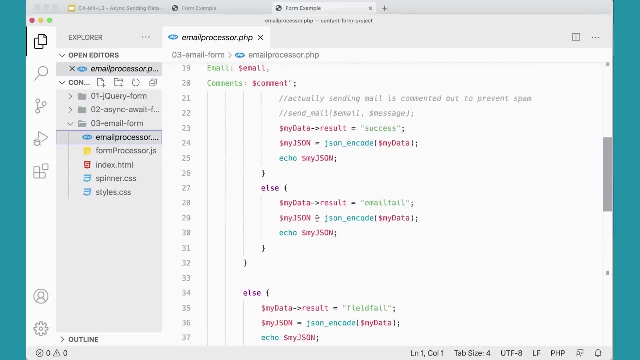 you would replace this with your email address that you want it to send. it want the form to be sent to that somebody fills out, So you would change that And then up here, the other thing you would have to do is that you would have to uncomment this line. 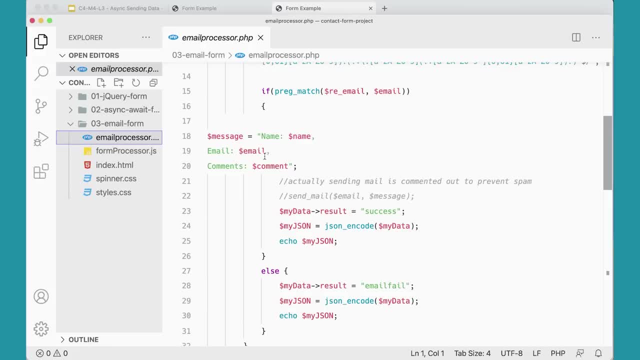 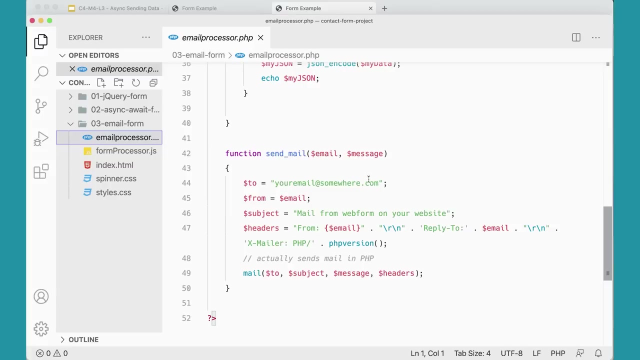 This send mail puts in the email, puts in the email address and the actual message and actually sends it. So that runs this function: send mail down here and that's commented out. So it's not actually going to send any messages because we don't have an actual address here. 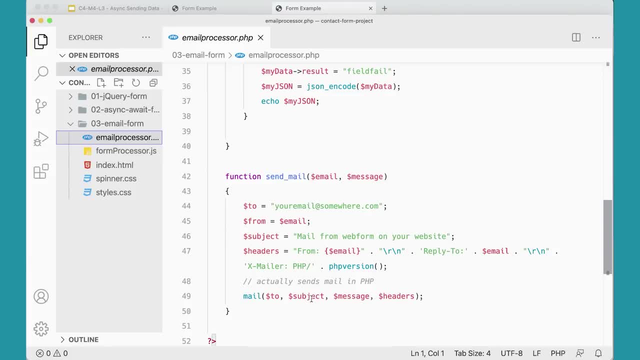 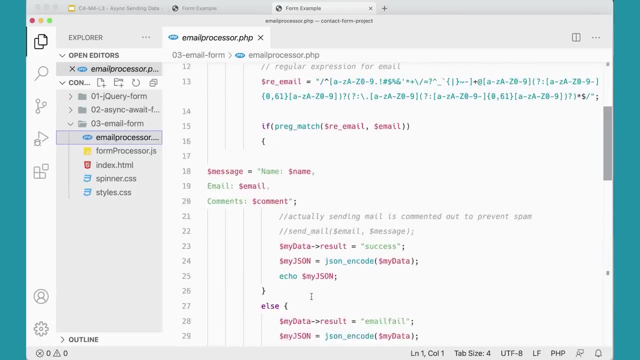 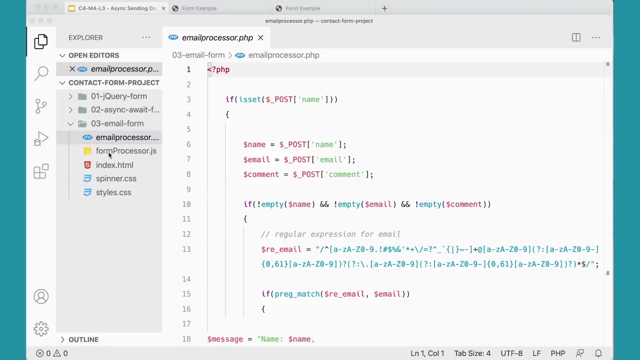 So this is a little bit hobbled for the moment for the purposes of this lesson, but you could use this file on your server if you wanted to, when you're done with this project, if you have a server to run it on. Let's take a look at the script file. 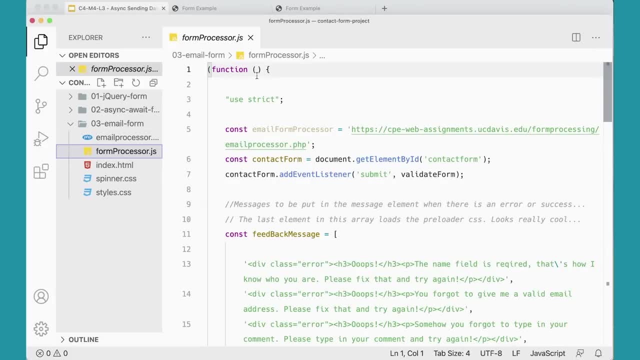 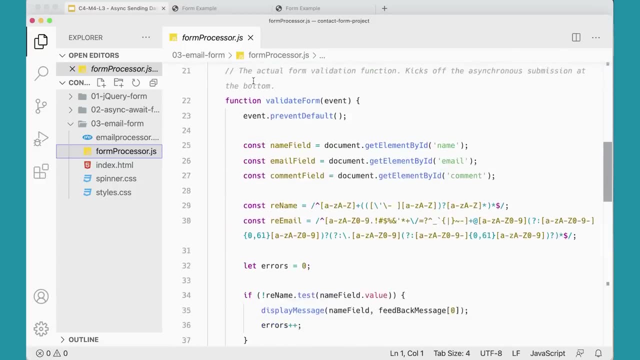 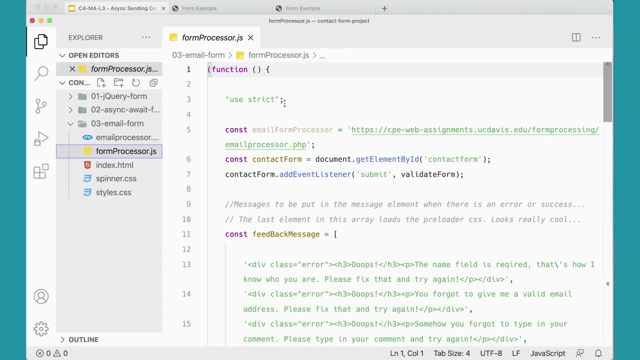 At the top of the script file you'll notice I'm using, I've got my IIFE, my immediately invoked function expression, and everything is inside of that. So that's all our best practices there. And then I'm using the use strict directive. 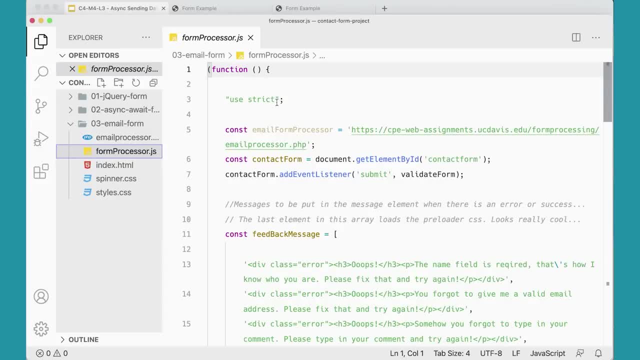 to make sure that the variables don't end up in the global scope by accident. And then here is the actual URL we're using, and it's the same one we were using before, except this last thing. here is we're using this email processor PHP. 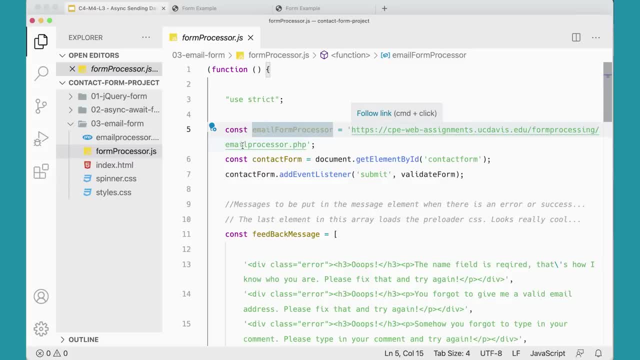 rather than just processorphp. So we've got that processor up there. Once again. we're getting our contact form, same as we did before. Once again we're capturing the submit and running the validate form And I've got the validate form. 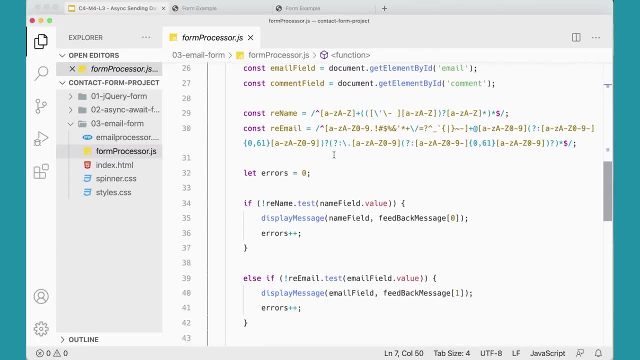 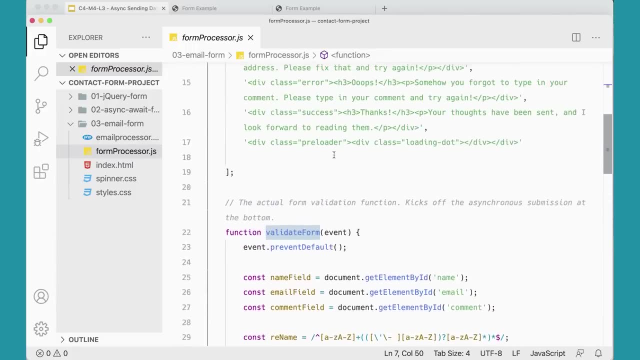 right here down here. This hasn't actually really changed much from before. There's slightly different fields, but it's a little bit different. We'll talk about how it's a little bit different. I've got an array here of feedback messages. 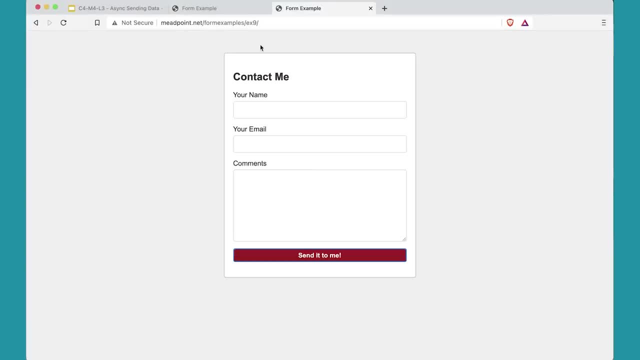 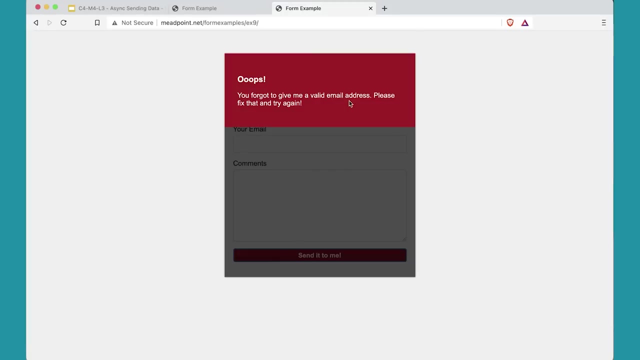 and these are the different messages that will come up on your form over here: Send email: Oops, so that's one message. If you put in a name here and then try it again, you'll get a different message for the email address, and so on and so forth. 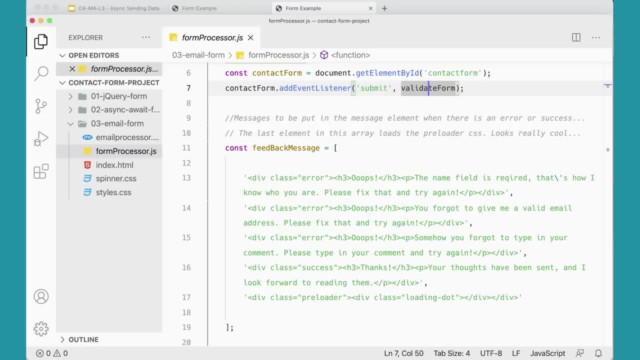 So we've got these different messages in here: Div class error. So the error is red and I've got a success one that's green. Oops, the email field is required. Oops, you forgot to give me a valid email address. 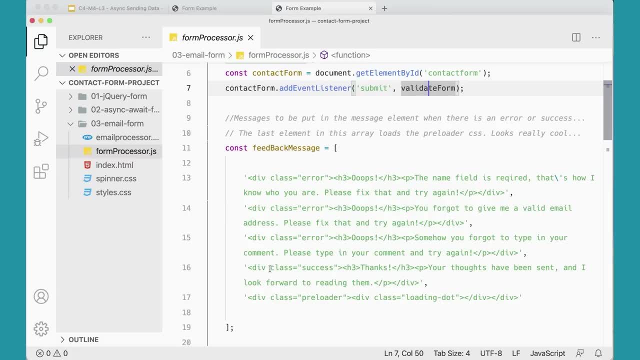 Oops, somehow you forgot to type in your comment. And then success. thanks, Your thoughts have been sent. I look forward to reading them. And then, finally, this one's the preloader that loads the animation of those dots that you saw when we ran the script earlier. 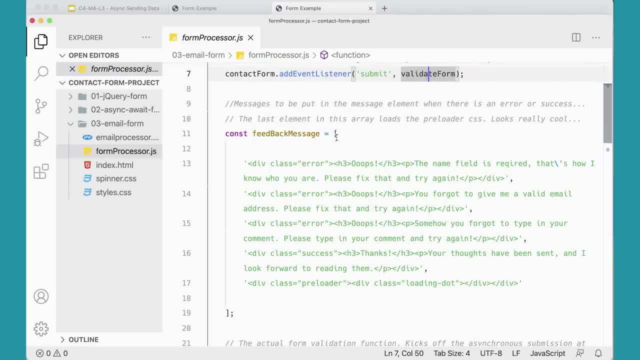 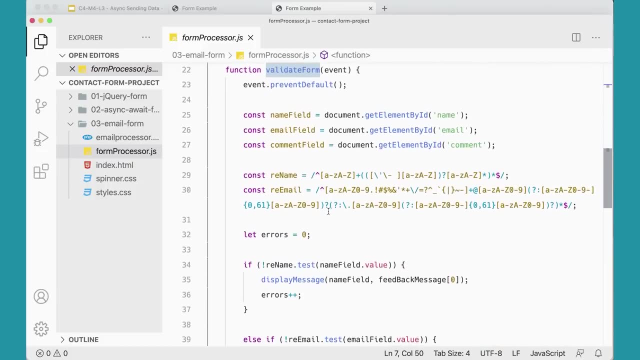 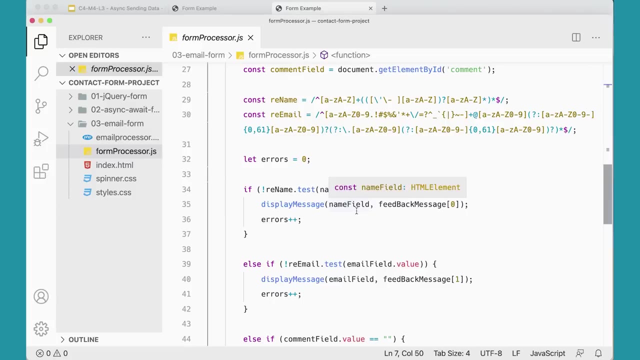 So this feedback message is an array that we'll be accessing to show the correct message And down here in the validator you'll see that we're going to run this function display message where we pass in the field that we're checking and the message that we want to display. 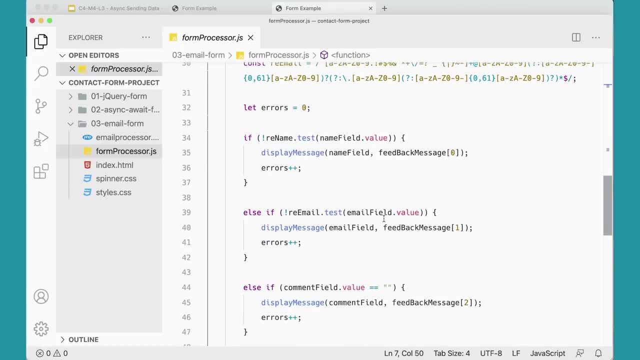 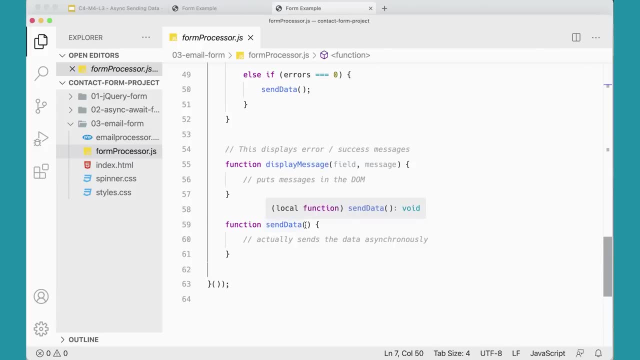 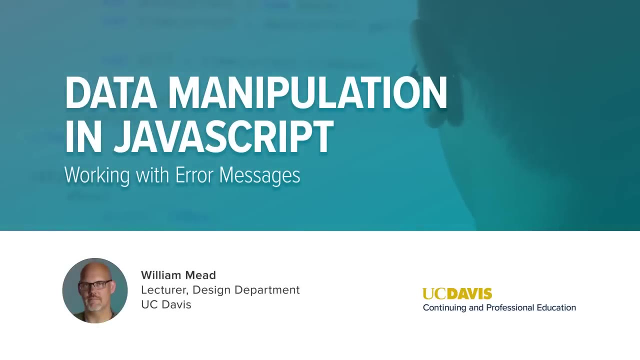 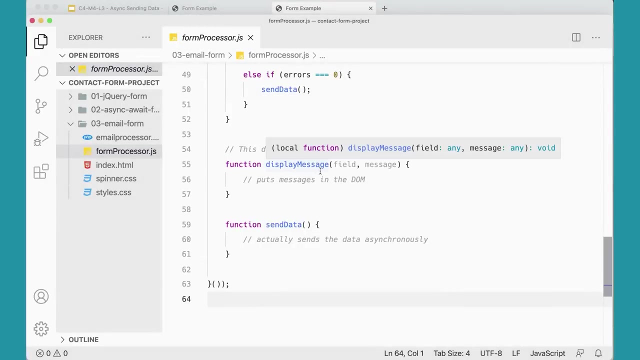 if it fails. So we'll be working on filling out this display message function here and the send data function here. Now that we've gone over our files, we can start working on our display message function here. So let's get started on that. 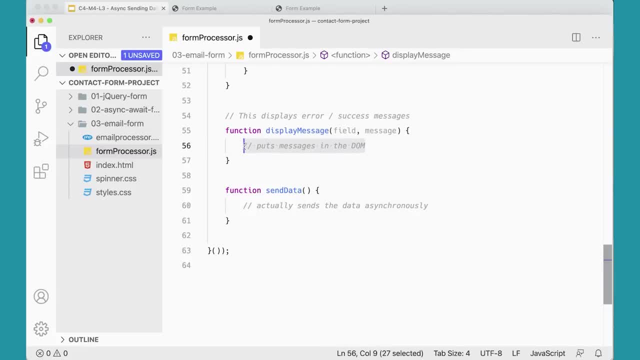 The first thing we want to do? let me get rid of this comment. I'm going to paste this in so you don't have to watch me type it, but you'll have to type it. The first thing we want to do is go get element by ID message. 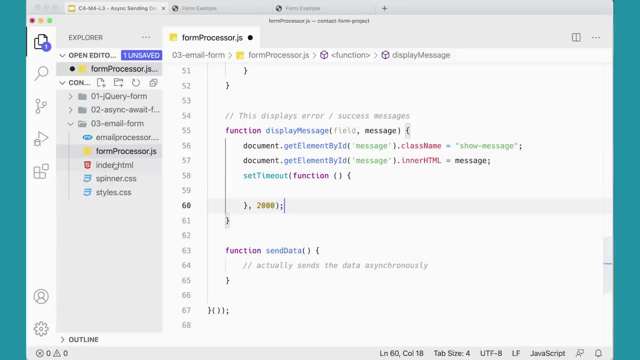 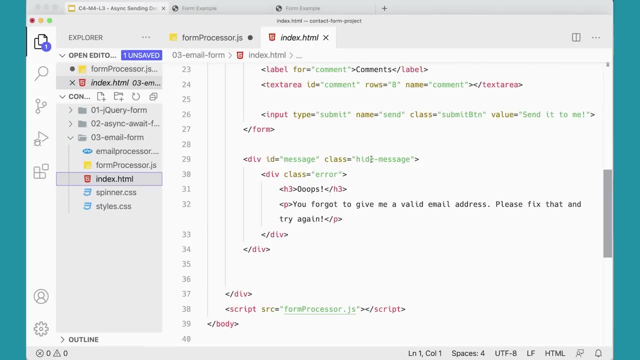 and set its class name to show message. What is that doing again Over here in our HTML? remember I mentioned that we have this div with a message in here and currently it's set to hide message. So we're going to set it to show message. 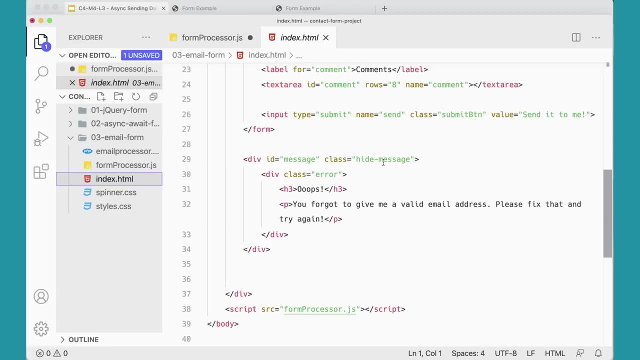 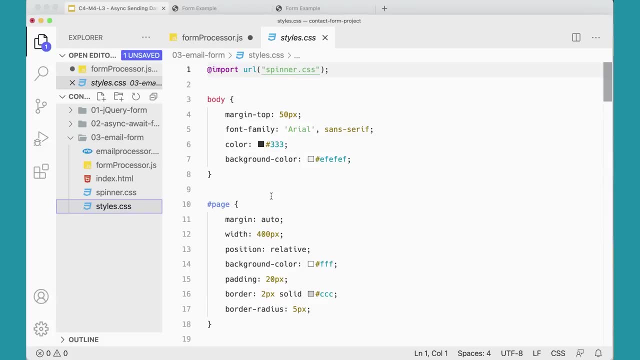 and that's going to make it go from being display none to setting it. so it's displayed And if you were to go over to the styles, you'll see in here there's already a style called show message. Here it is display block. 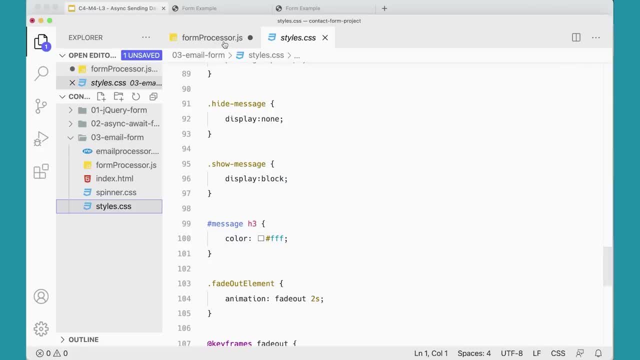 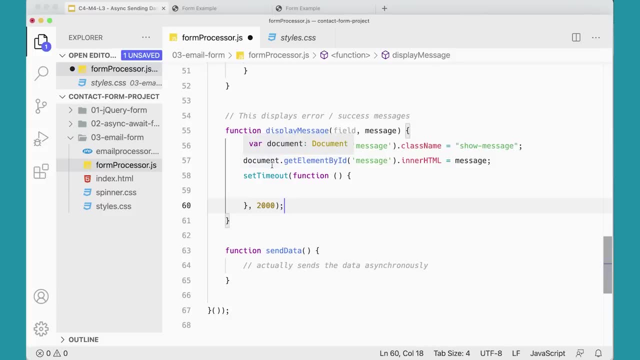 So that's going to show that message. It's going to change it, so it's set to show message, And so then it's going to show the message and then we're going to say, okay, get that message element again and change its inner HTML. 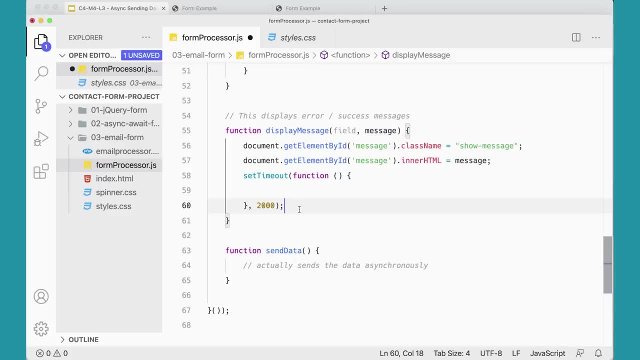 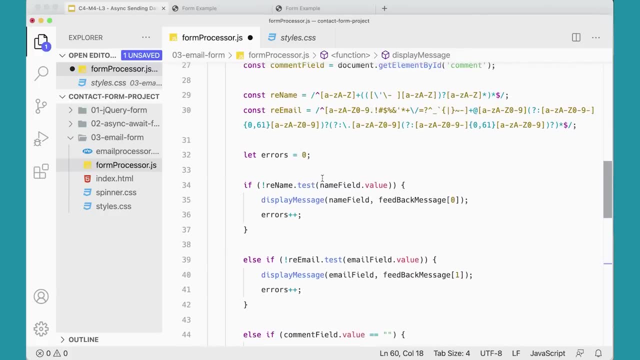 to whatever message gets passed in here, And then we'll talk about the set timeout in a minute. But what is this message that gets passed in here? Well, up here, if you didn't fill out the name, the message that gets passed in is feedback message zero. 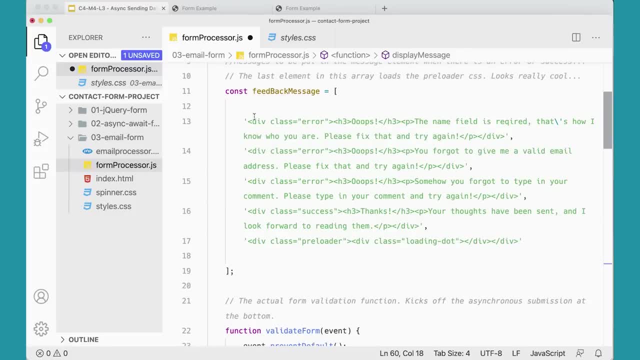 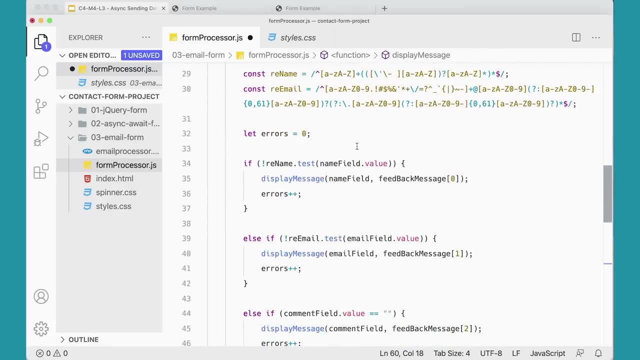 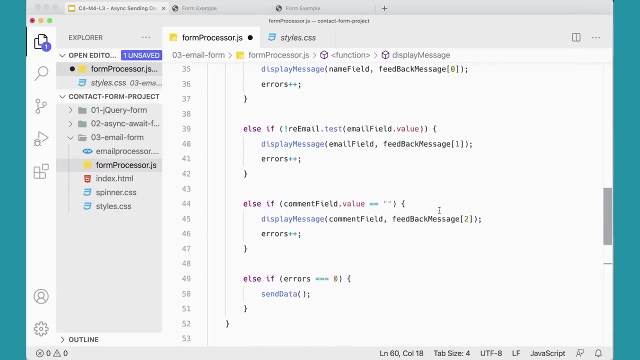 Come back up here. Feedback message: element zero is oops. the name field is required. So each time we run this function we're passing in a different element from the array, depending on which message we want to show. So that's going to be the inner HTML. 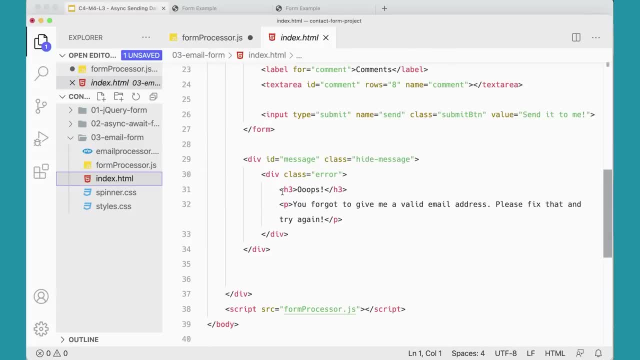 this div over here. It's going to get replaced with a new div with the correct one in here, And I have one of them in here, but that's just going to get removed because we're doing inner HTML in this message div, So it's going to take everything out of this div. 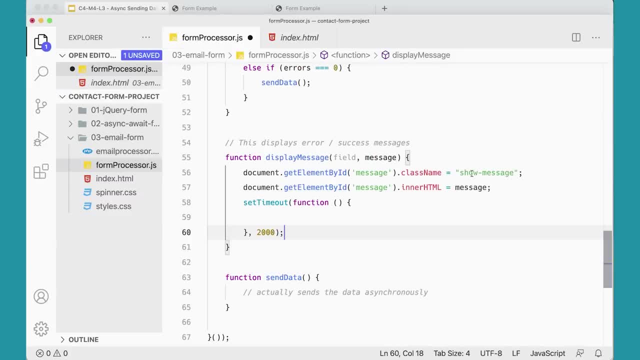 and put in new content. And the new content it puts in is the content from up above, So that gets put in, So it's going to get put in, and then we're going to wait two seconds and then fade it out. So if you come over here, 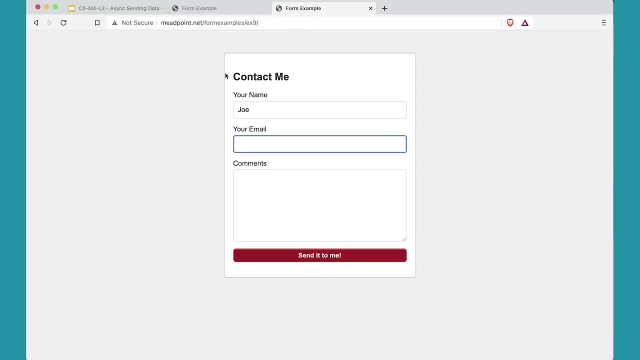 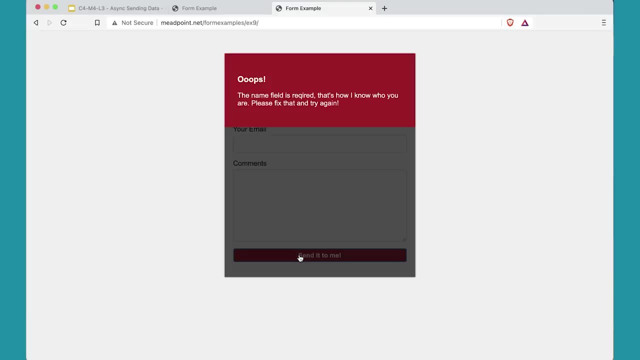 we're going to look at the finished version again just for a second here. If I refresh that, if I forget to put something in here and click send it to me, it makes the message show and then it's going to fade it out. 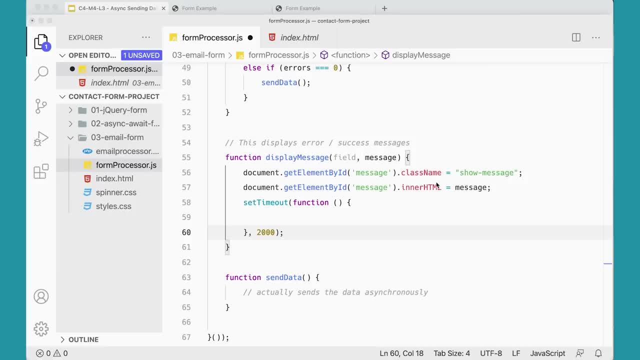 So it puts the message on the screen and changes it. so it's showing and we're going to leave it on the screen for two seconds. We can make it longer if you wanted to. You can change this to something longer if you felt like you needed more time. 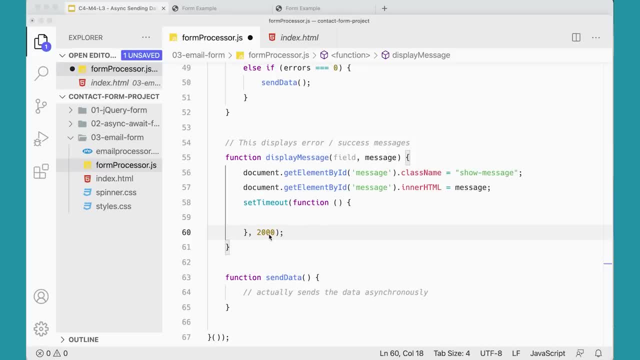 to read those messages, But we're going to leave it on there for two seconds. When those two seconds are over, we're going to fade that message out. like this Document: get element by ID message: class list: add- fade out element. So we're adding to the list of classes. 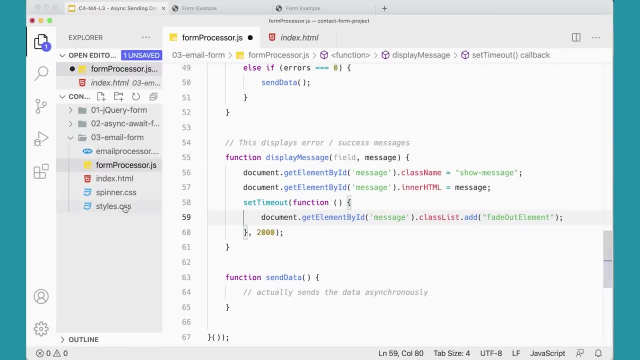 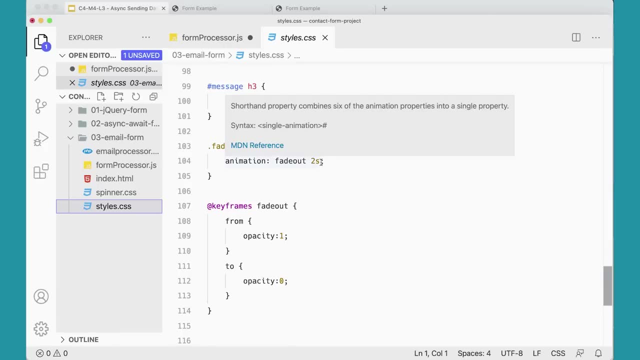 a class called fade out element. And again, if you come over here to the CSS and look down here at the bottom, you've got fade out element which runs an animation over two seconds. So it's going to take two seconds. 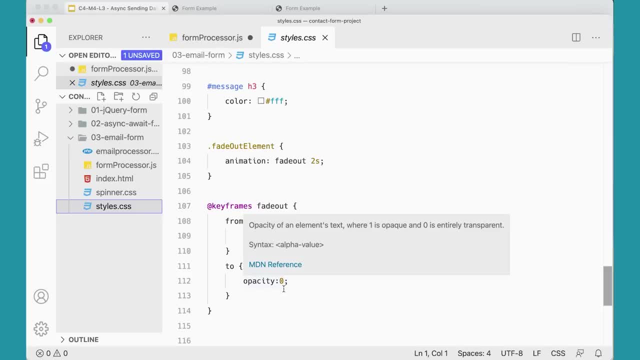 for it to go from opacity one to opacity zero. It's still on the screen, It's still showing, but it's set to an opacity of zero, So you're just looking through it And after that's over. so now we've got to wait two seconds. 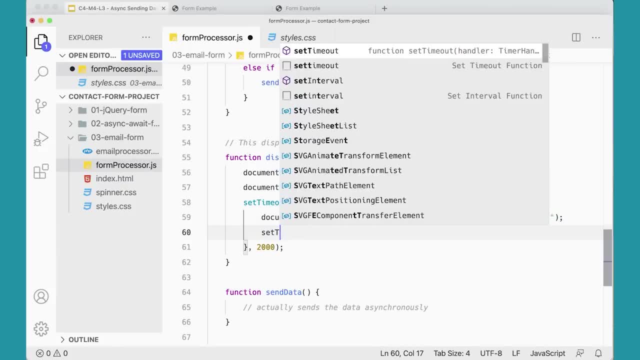 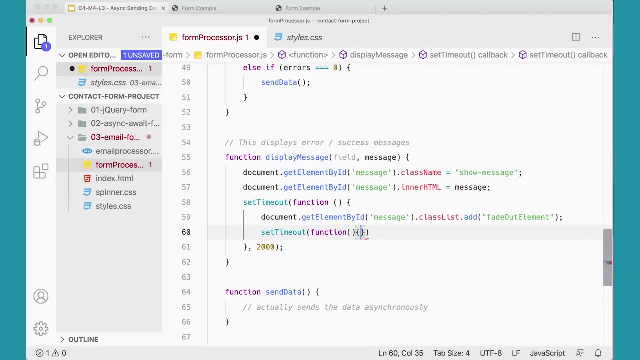 before we do the next thing. So I'm going to do set timeout again here. Set Timeout: I'm going to run a function And that function's going to happen after two seconds. Okay, Because it's going to take two seconds for it to do this. 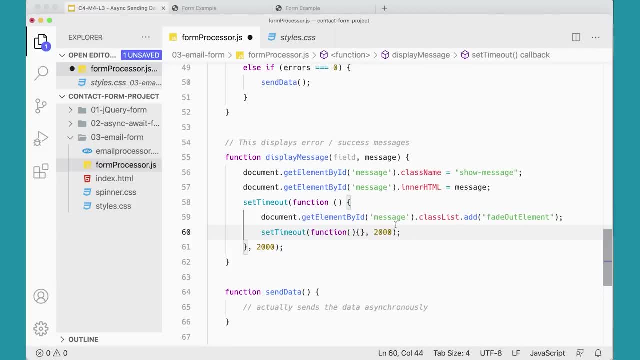 I need to wait two seconds before I do the next thing. I could do an event listener for listening for animation end, but this seems like a pretty expedient way of doing it. I know that it's going to take. this is going to wait at least two seconds. 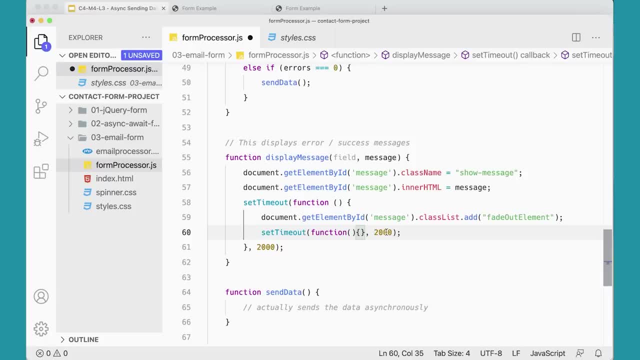 maybe even a little bit longer if necessary, But I just need to wait until that thing is actually faded out. And then what do I want to do? I want to set it back, so that it's now invisible. So I'm going to do this again. 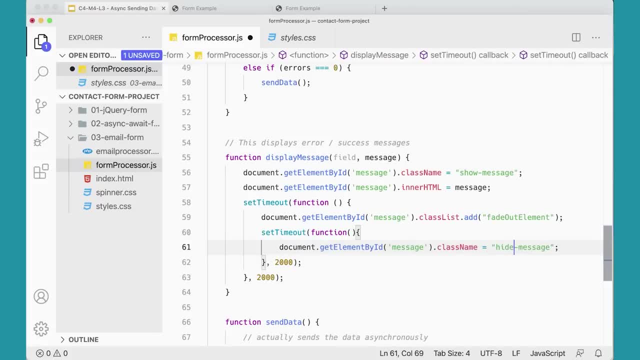 But instead of show message, I'm setting it back to hide message So that the class name just goes back to what it was before. And this is very typical when you're working with interface elements: is you start in one sort of place? 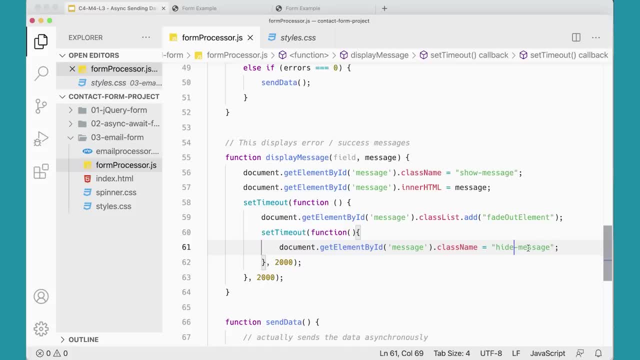 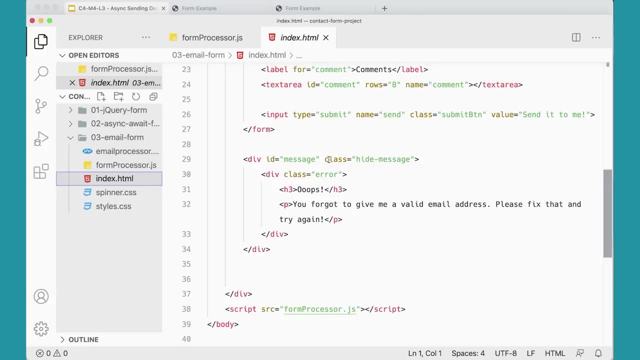 you make some changes and eventually you want to bring it back around to the state it was in originally, in its original state, And the original state here was that the class was set to hide message. So once again we're showing the message. 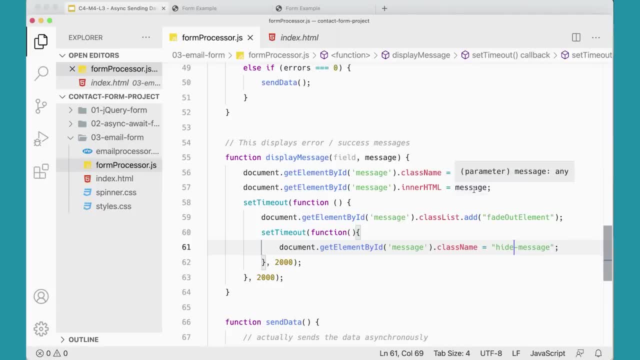 we're. we're making it so that it's displayed, setting the message, waiting two seconds, fading it out, waiting two seconds after it's done fading, fading out and setting it back to hide message. The last thing we need to do is 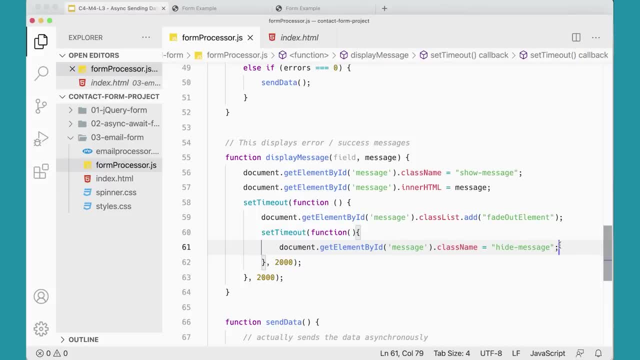 put the cursor back in the field that they forgot to fill in. So I'm going to do that like this Document: get element by ID field. field is getting passed in here And we want its ID And we're going to use the focus method. 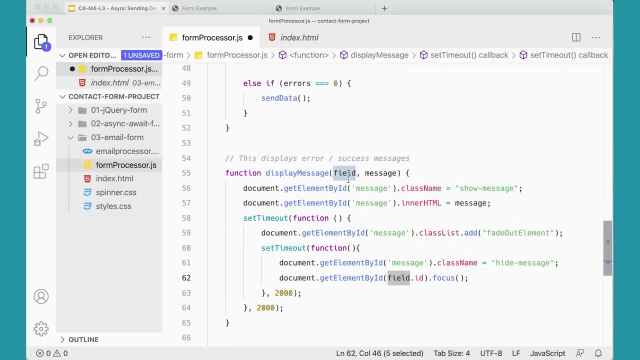 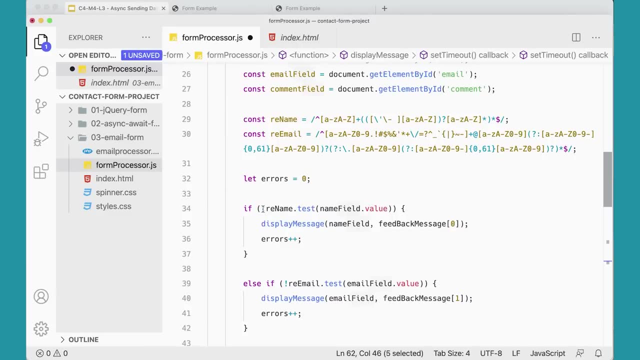 to put the cursor in that field. So again, what is that field? If I come up here and look at this, if, if it doesn't pass the, the test for the name, not re test. name value. display message. name field. 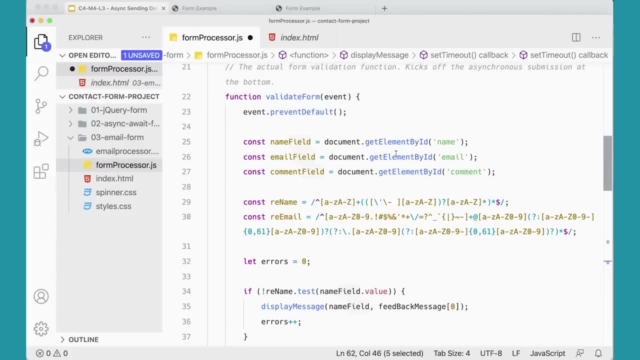 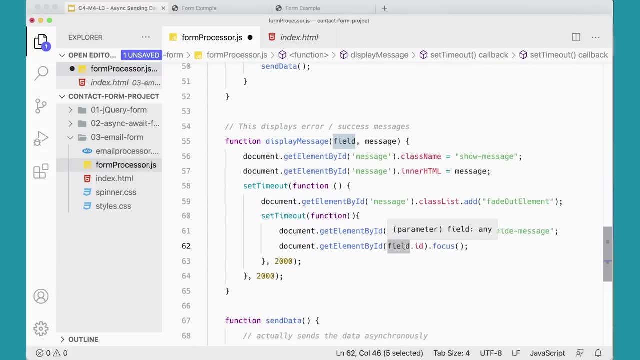 So what's name field Document? get element by ID name. So I'm I'm getting all of this stuff. You can see how it kind of piles up here, Getting that element by ID name, but I want its ID And then I want to focus on it. 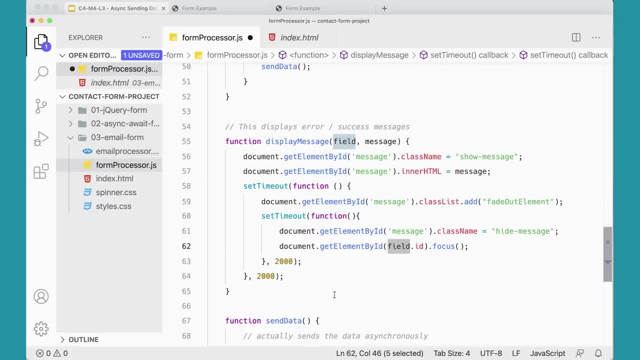 And that should actually work. And I'm not going to really test this yet because because we need to do a few more things first, But actually we should be able to test this. I think If we come over, we're not doing any success yet. 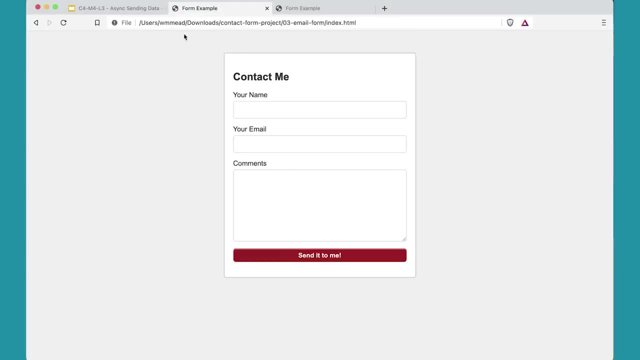 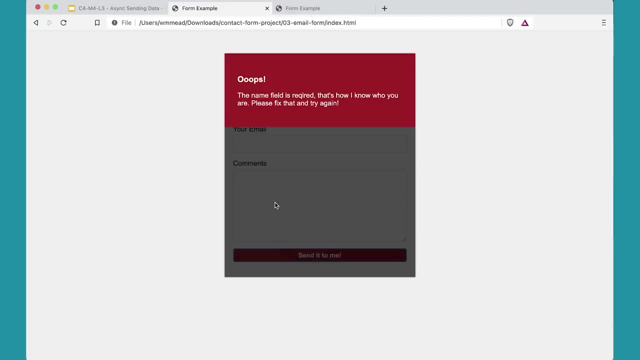 It should work If we come over here. So this is the local one that I have in my downloads folder. I'm going to refresh it. If I don't fill in the name field, it says: oops, stays on for two seconds. 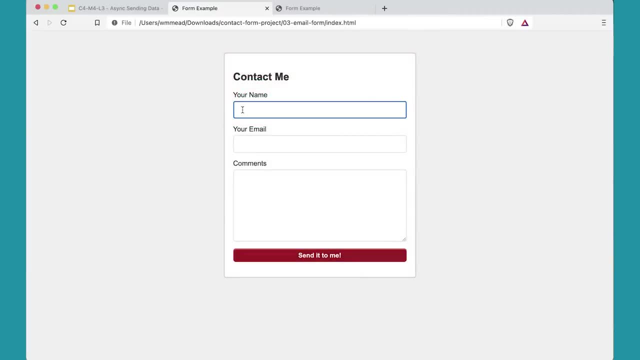 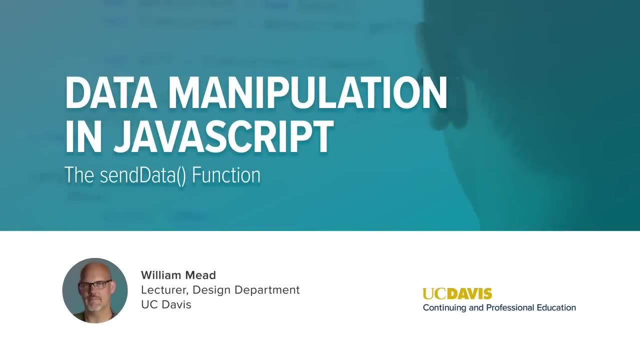 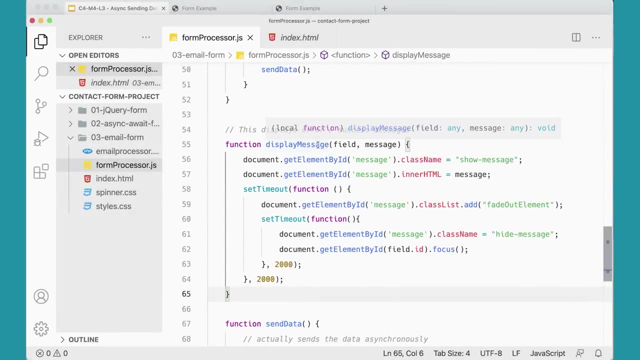 fades out and then puts the cursor into the field, So that's working perfectly. We are mostly done with our display message function. We're going to have to adjust it just a little bit in a few minutes to handle our success message as well. 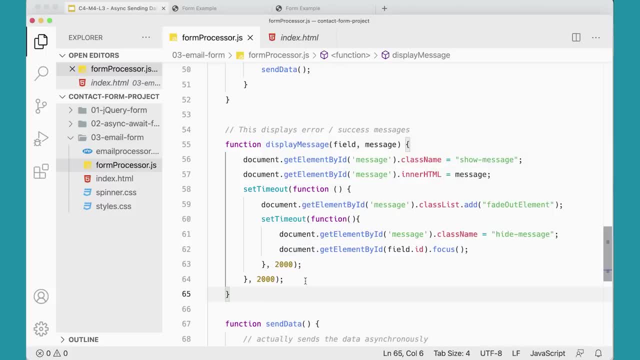 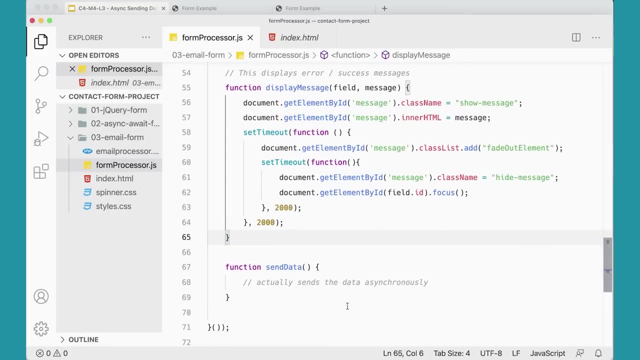 But we're mostly done with our display message function And now we can work on filling out the send data function, And this function is going to look very similar to what we did in the previous exercise. We got to do a little bit more. 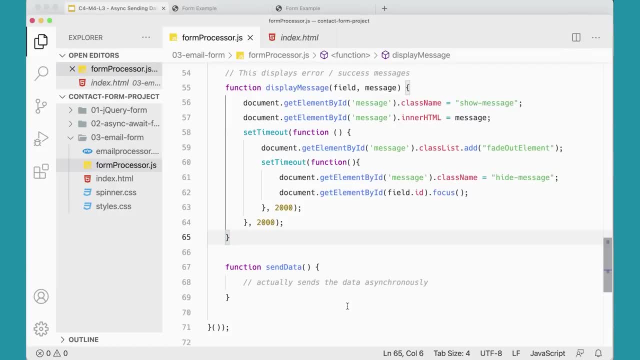 to sort of handle the interface that we want to happen and have come up. But other than that, it's very similar to what we've, what we've done before. First, we'll show the message by setting the class to show. 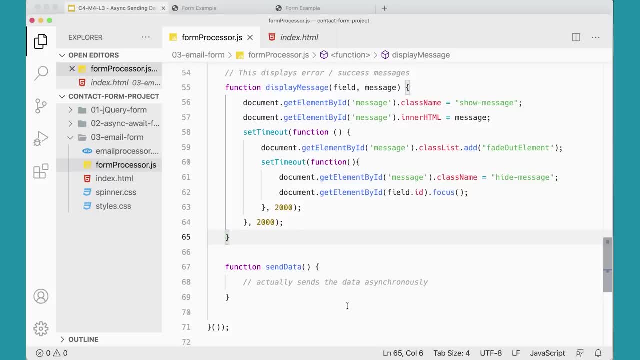 to show message and add the feedback message for- which is the really cool little spinner thingy- And then, regardless of how long it takes for the server to respond, you want the spinner on the screen for at least two seconds. It might take longer, depending on. 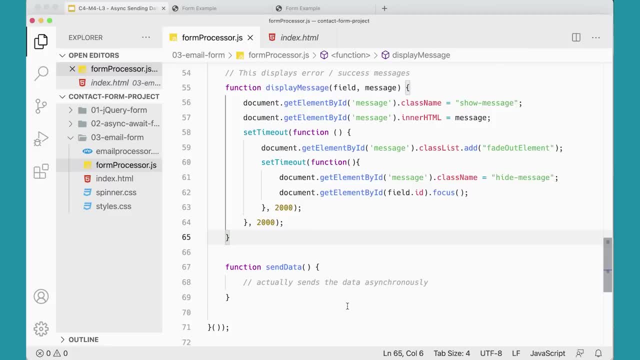 if you need to wait for the server, but we'll have it be on the screen for two seconds at least, And when the two seconds are up we'll do an asynchronous function to send and get the data. So let's start putting this into place here. 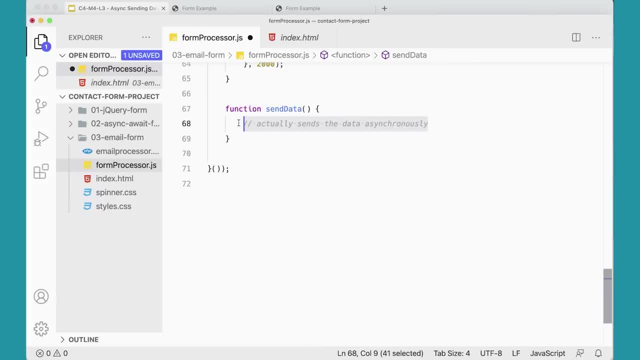 I'm going to take out this comment. I don't really need that. And then the first thing I'm going to do- and you're going to have to type this, but I pasted it in here- I'm going to go get my element by ID message. 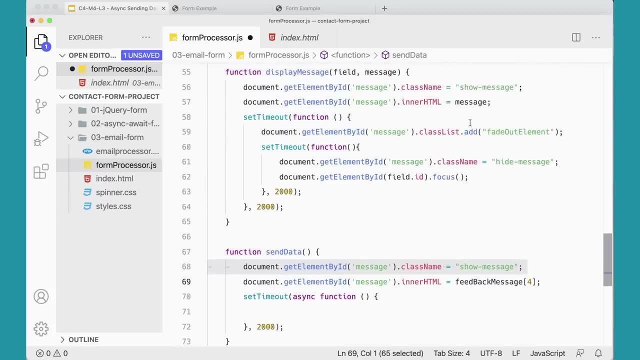 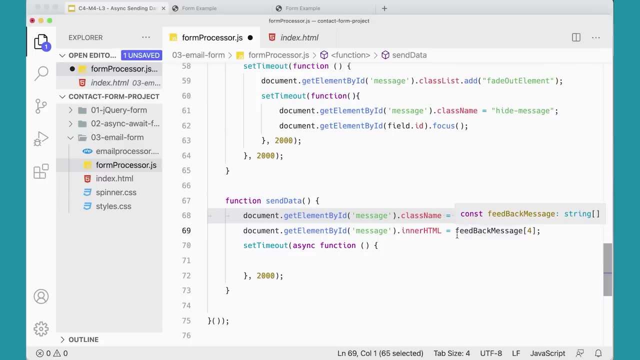 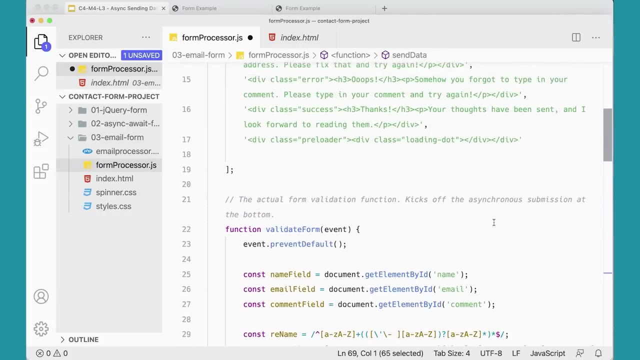 class name: show message. You can actually just copy and paste that from up here. It's the same thing. And then I'm going to set the inner HTML to five And then the feedback message, square bracket four, which, again up here, is our last one here. 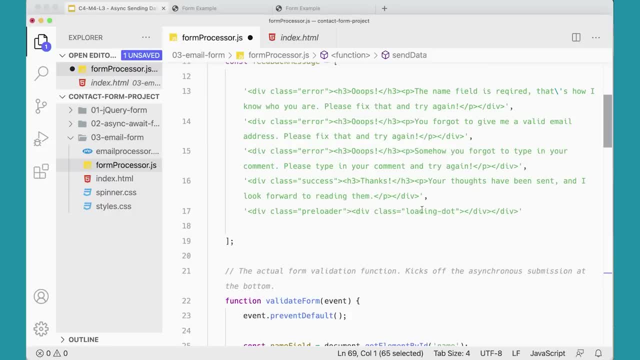 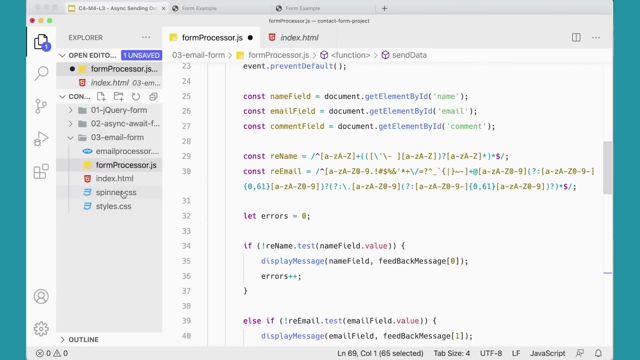 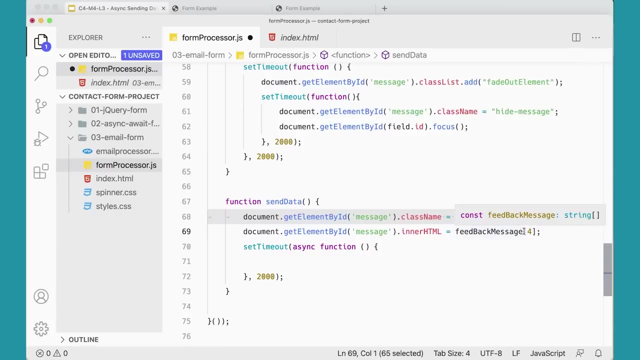 Zero. one, two, three, four. Preloader: the class loading dot. It's actually a div inside of a div that creates that animation, And go look at this spinner CSS to see how it actually works, if you want to. So yeah, so that's going to be set to feedback four. 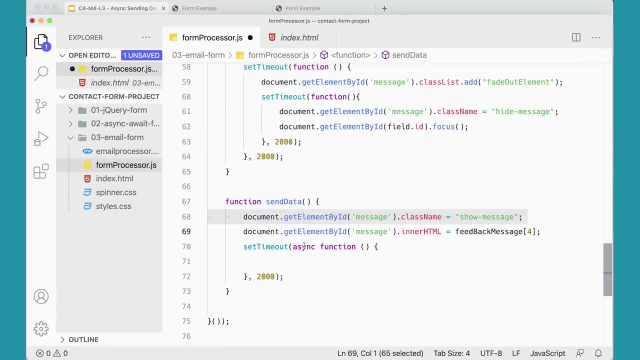 And then I'm going to run setTimeout, which is going to run a function, But now I'm sticking async in front of that function because this is going to be an asynchronous function. I want to wait at least two seconds. I want the spinner on the screen for at least two seconds. 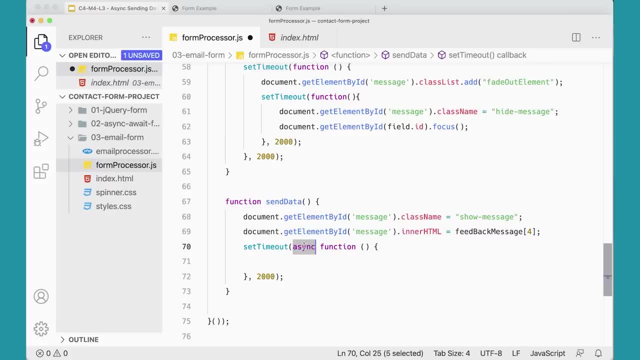 because it kind of looks sort of cool And so you can see it for two seconds. That's quick enough that you can see it, but not so long that you're going to be annoyed by it. Two seconds goes by pretty quickly. All right, great. 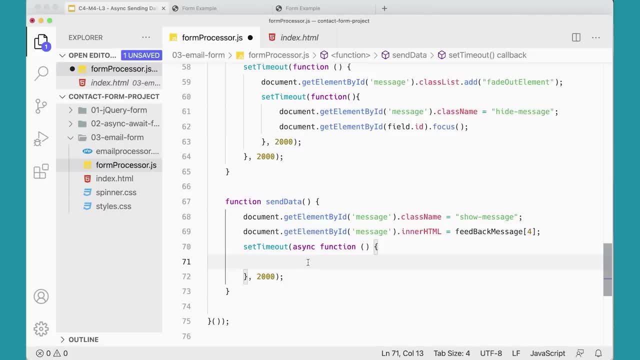 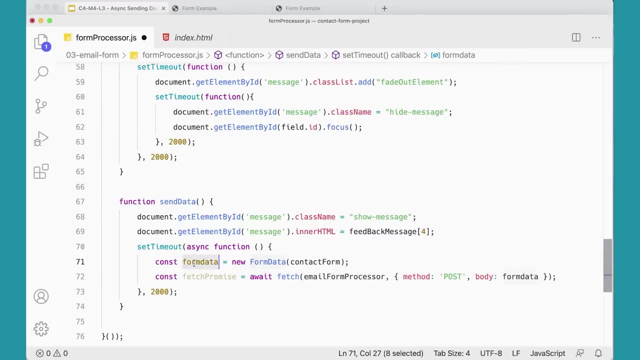 So now in here we're going to do our asynchronous functions for sending our form data. I'll close this thing so it's always easier to read here. But again, form data is what we're using, So this is exactly what we did before. 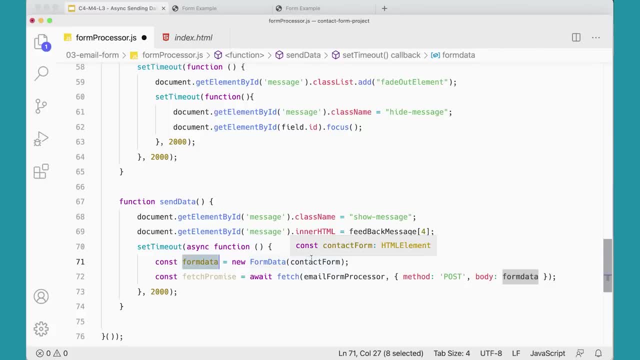 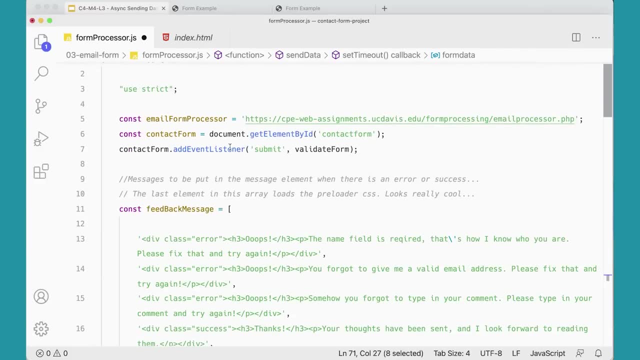 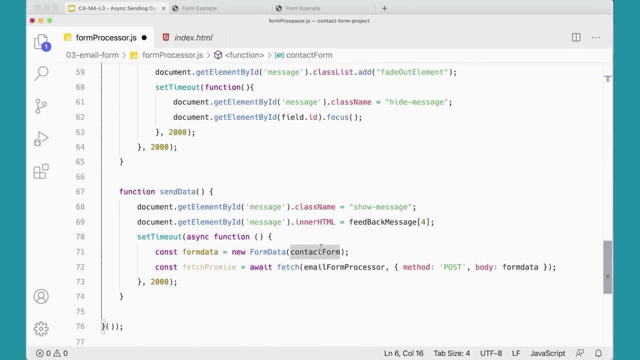 Contact form is the actual form that we have. This was defined up here at the top of the page: Contact form. Oh, there it is. Document get element by ID: contact form. So there it is. So we're getting the contact form. 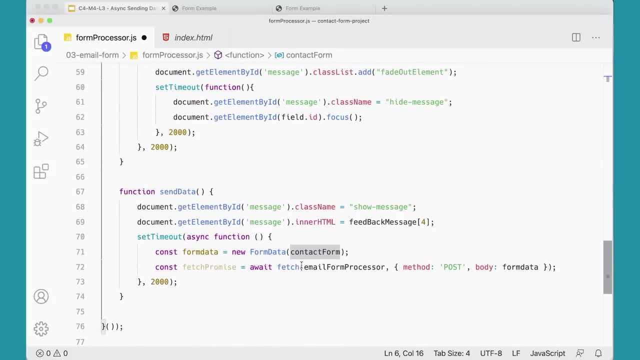 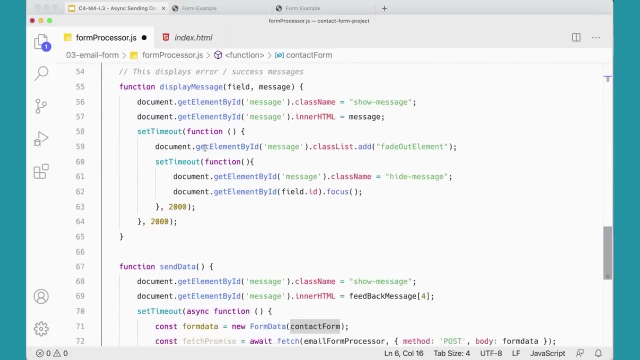 And again we know by the time we get here that it is past the validation, because the send data function only runs if there are zero errors in the form. So that's all good. And then we're fetching and we're using our await keyword that we can use. 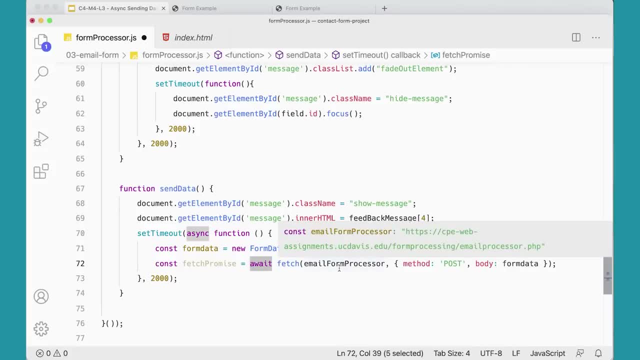 because we put the async there And we're doing the same thing we did before, except now we're getting email form processes. So this is our email form processor, which is our email form processor. We're sending the post. We're sending by post. 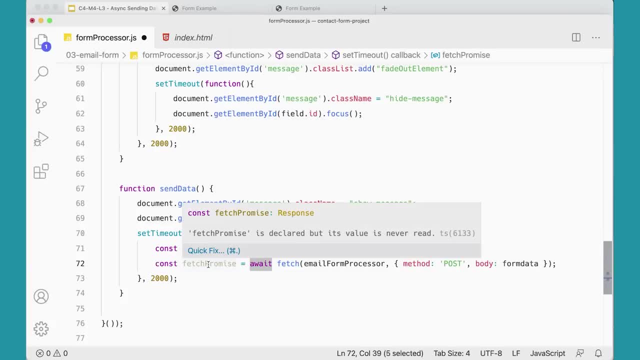 We're sending our form data that we created here, And we're putting all of this back into our fetch promise that once it has successfully done this, then we can go on to the next part. Let's add that in now These two pieces. 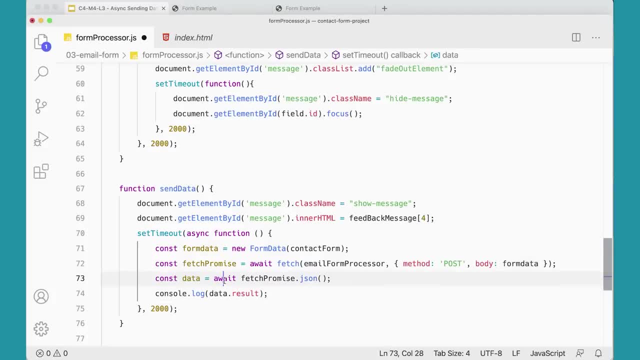 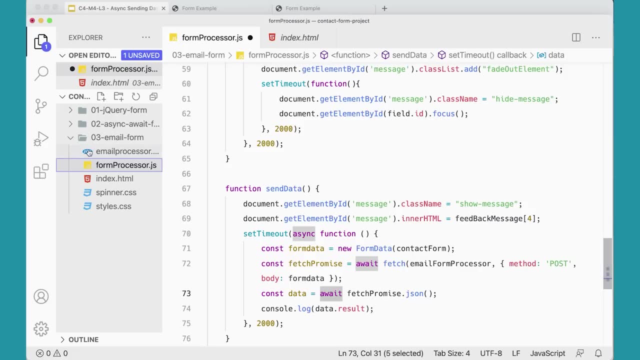 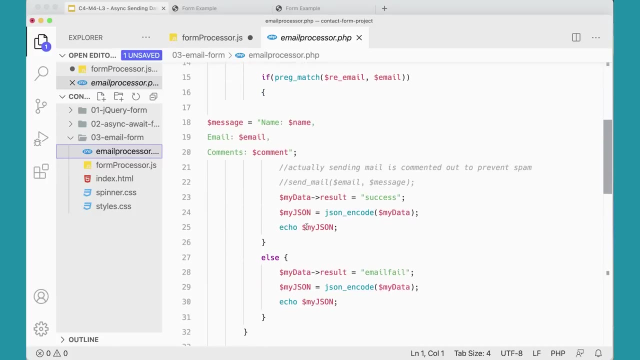 So I'm making a variable data, I'm using my await keyword and fetchpromisejson. And why is it JSON? Well, because, again, if you look at our PHP processor here, this thing is going to return some JSON. It's encoding some data in JSON format. 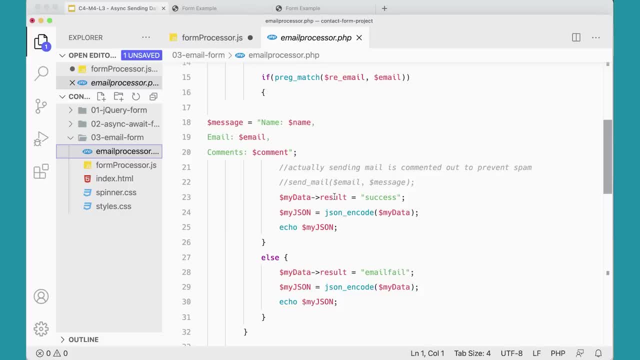 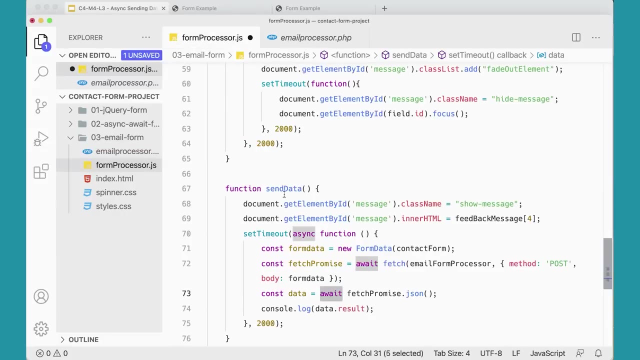 And it's going to either return a key value pair, that's result success or result email fail. One or the other is going to come back from this form. Hopefully we'll get success back And that's what we want to check for next. 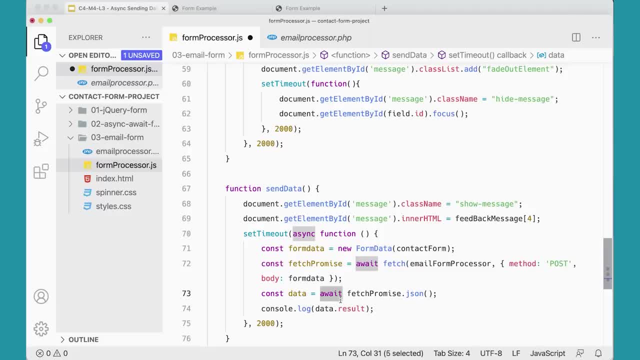 is. we want to check to make sure that we got success And I'm just console logging out here data result so that you'll be able to see it in the console log And we'll leave that here. I'm not going to check it just yet. 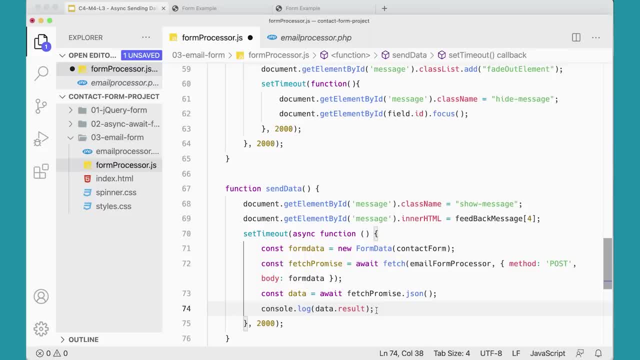 We need to do a few more things first, But we'll check it. But we'll check it there. So this should be getting our form data and doing everything we need to do. The next thing we need to do is show the correct message. 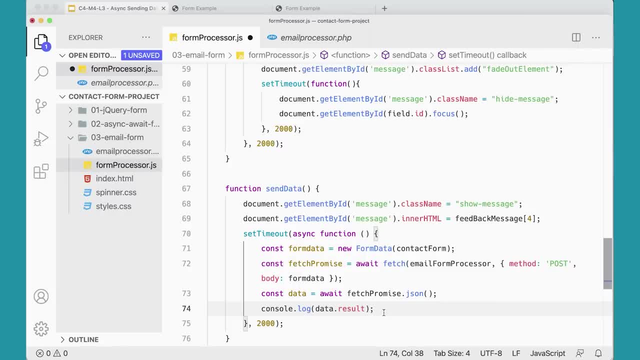 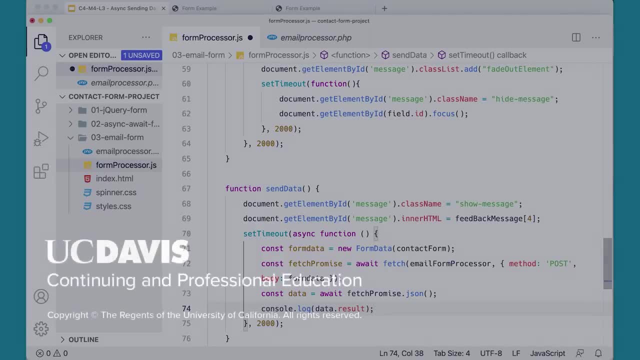 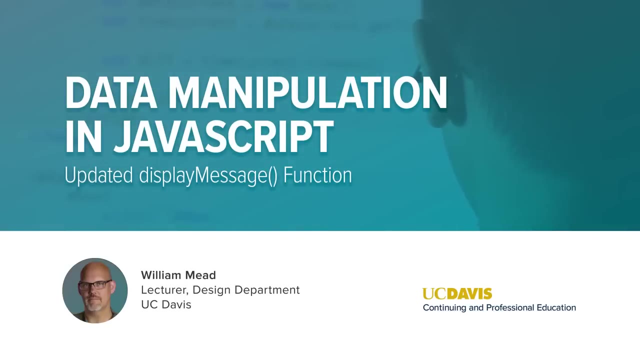 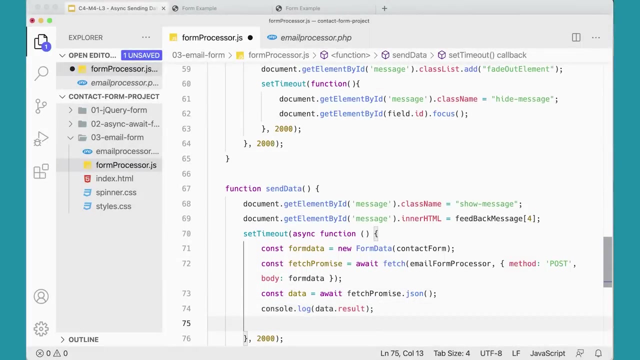 our success message And we'll have to modify our display message function a little bit for that, And we'll do that in the next video. We've got our send data function almost finished here. We just need to finish it up a little bit. 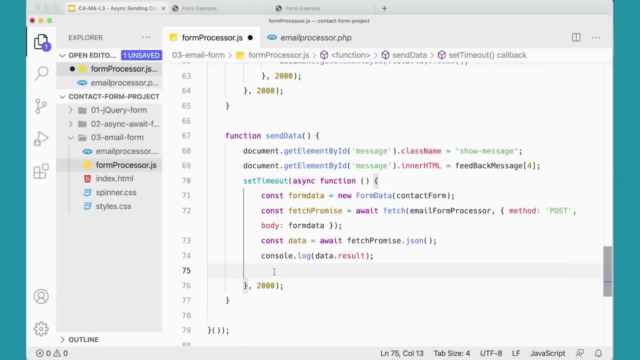 And all we need here is to set the message right, And what we're looking for is for this dataresult to be the value of success rather than fail. So I'm just going to put an if statement in here. If dataresult, that thing. 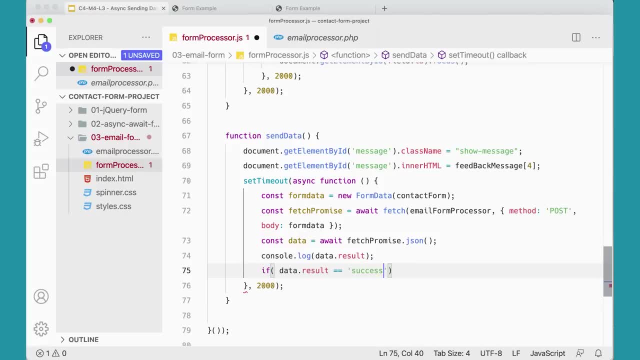 the same as success. What am I going to do? I'm going to do this: I'm going to run the display message function, I'm going to pass in success instead of a field name And then I'm going to pass in feedback message 3,. 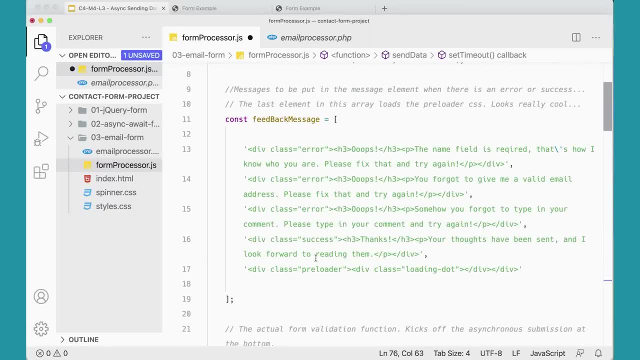 which again up here. if we go up to our feedback messages 0,, 1,, 2,, 3, div classes, I'm going to say success. Thanks, Your thoughts have been sent And I look forward to reading them. 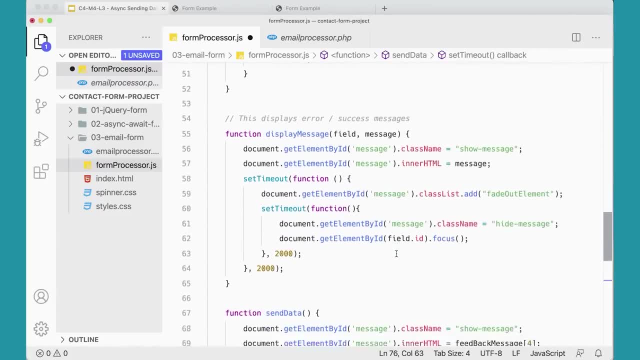 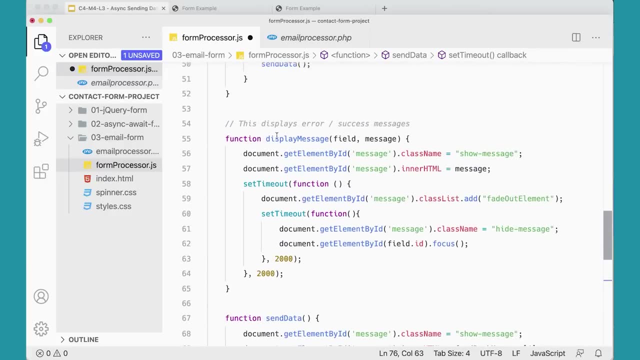 And we close the paragraph in the div. So that's what that's going to be set to here. Now up here, if you look at our display message thing, it's expecting a field in here. We're passing in instead the word success. 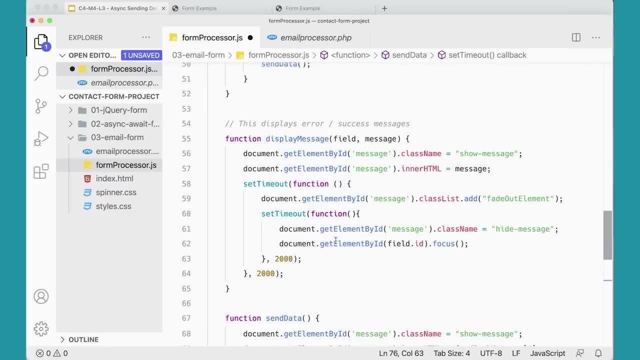 And down here. this is where we're actually processing this when we get down here. So what I want to do down here is I want to put an if statement, If, And I want to check to see if it's not the word success. 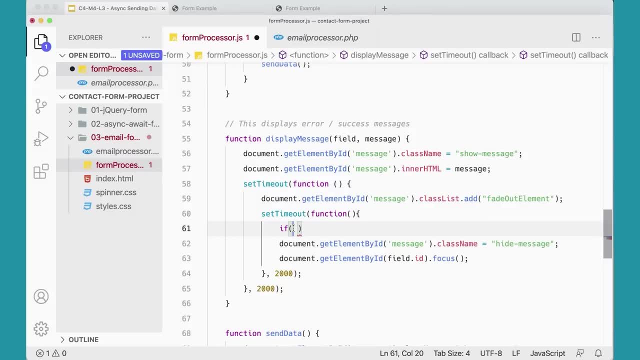 So if field- the value that's passed in there- is not the same as, not equal to success, If it's not that, then I want to do this stuff here, Like that. So if it's not success, then I want to do. 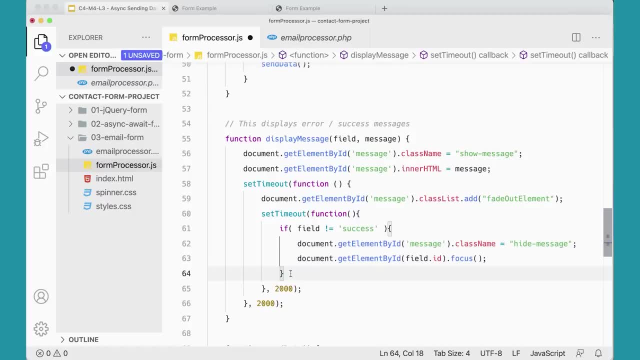 then it must be an error and I want to handle that. Else, Oh my goodness, Else. What do I want to do here? Well, I want to do this again. I just want to empty out, I want to set it back to message. 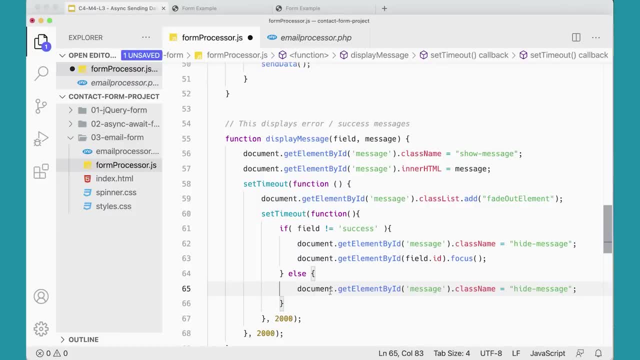 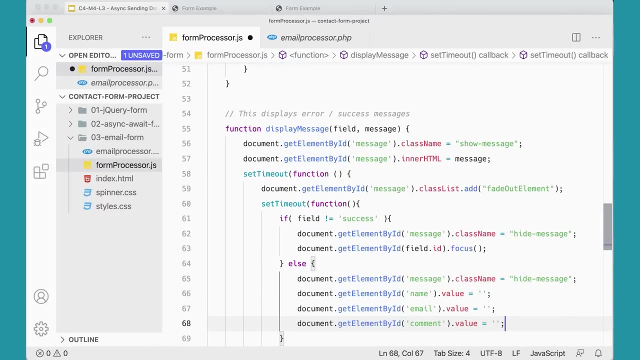 Probably could have put this outside the if-else statement, So I only have to run it once. So I want to do that, And then I want to clear out the fields. Previously, in our previous example, I wrote a fancy little loop to clear out the fields. 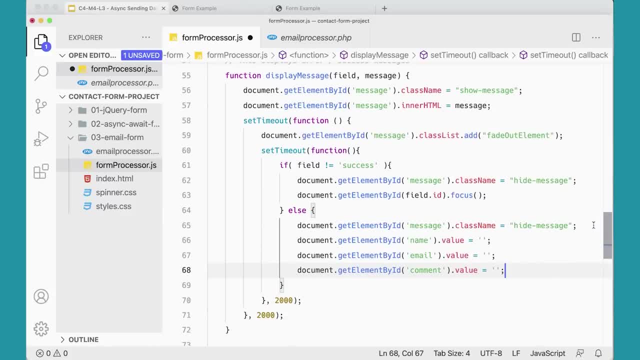 But here we only have three fields, So I'm just going to do it in sort of a lame way and get each one of them by ID and just set the value to empty. Since there's only three of them, it's not that big a deal. 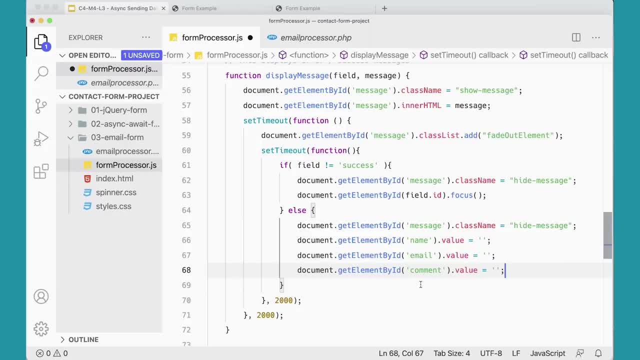 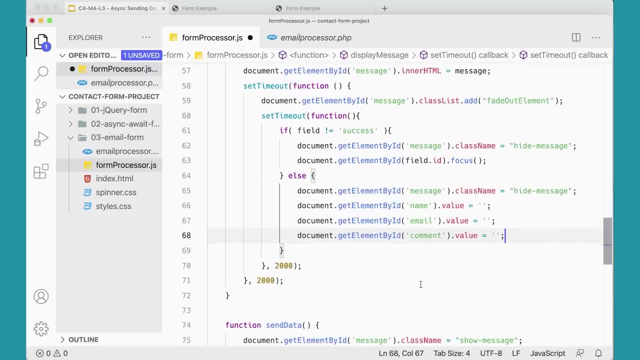 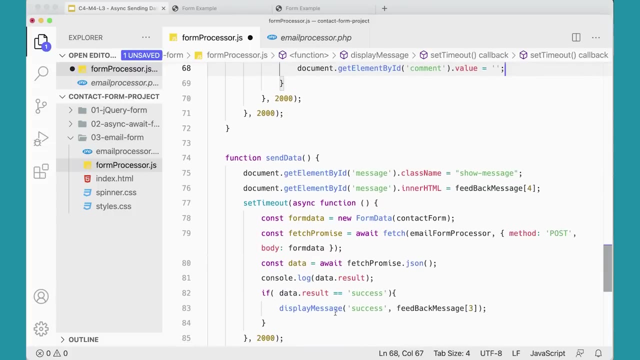 You could do a loop here if you wanted to and loop through them and do all that fancy stuff if you wanted to, But this seems to be fairly good. So now what happens is that when we run send data, assuming everything works well- we're going to use the display message function. 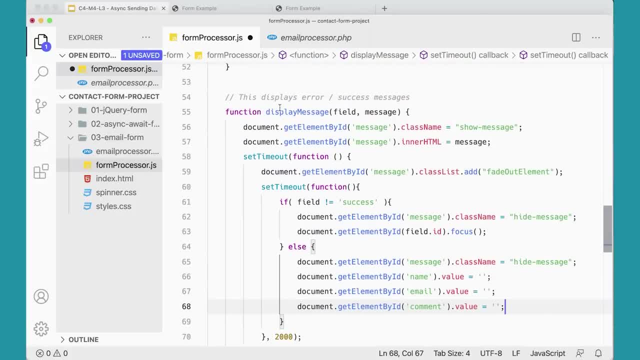 to display the success message. So this display message function says it's taking a field here, but sometimes it's a field and sometimes it's the word success. If it's a field, it's going to do the error, because there must be an error in the form. 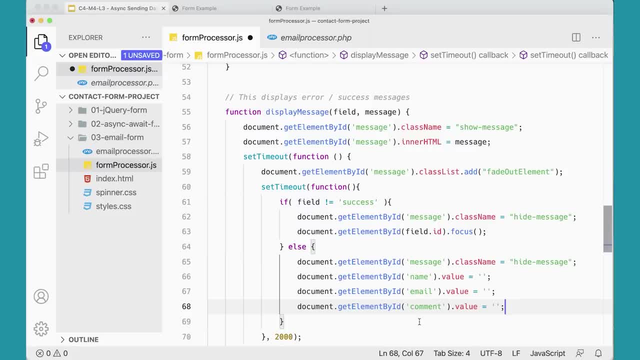 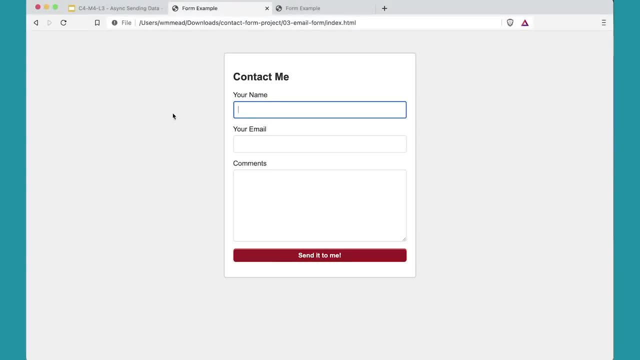 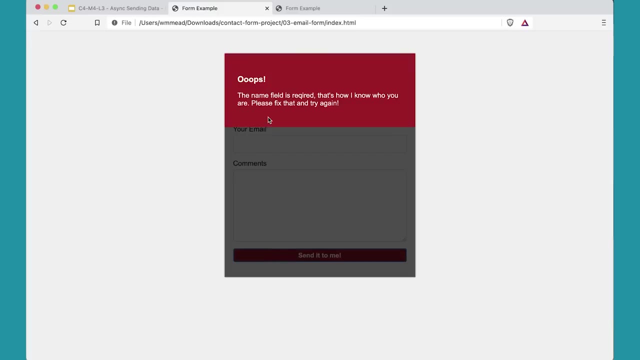 If it's success, then it's going to give us the success message. Hopefully that'll work. Let's give it a try. Come over here and I'm going to refresh my page And if I just click send it to me, I get my error message. 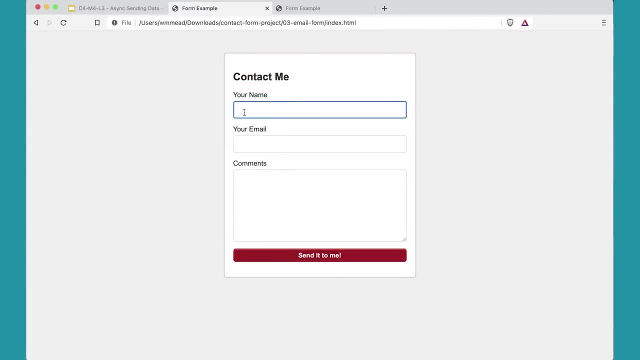 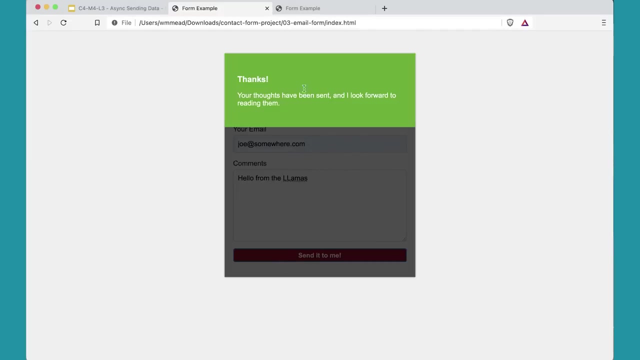 It tells me I need to fix my form. It puts my cursor in there. I'm going to do Joe, Joe at somewherecom, And then hello from the llamas. And if I click send it to me, I get the little spinny thing for at least two seconds. 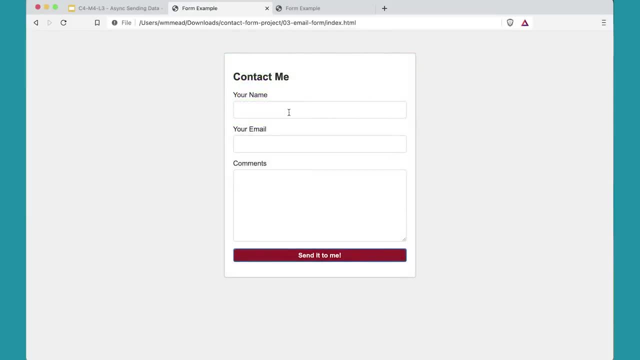 And then, once that's done, I get the green message that says successfully sent. And when that's done, it fades it out and I'm all the way back to where I started, And that's perfect. Now, also, if I click inspect, 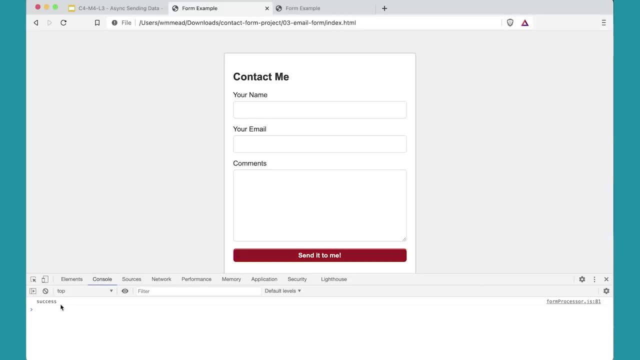 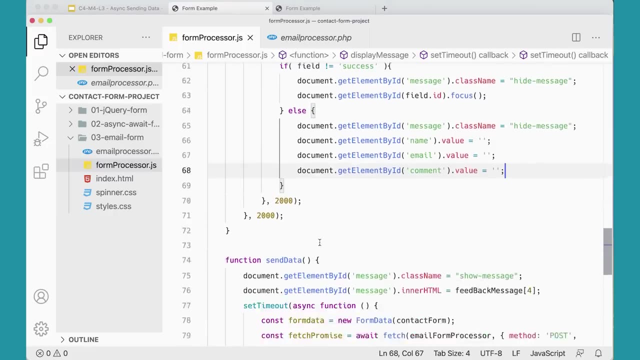 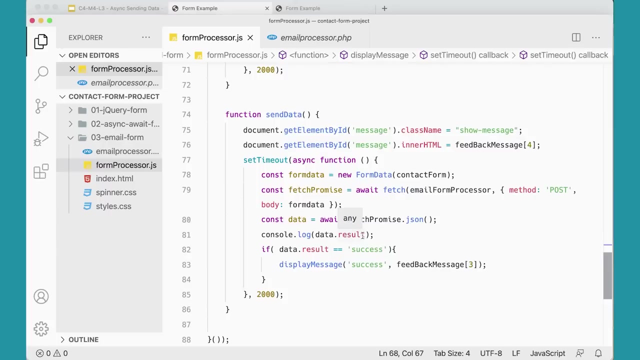 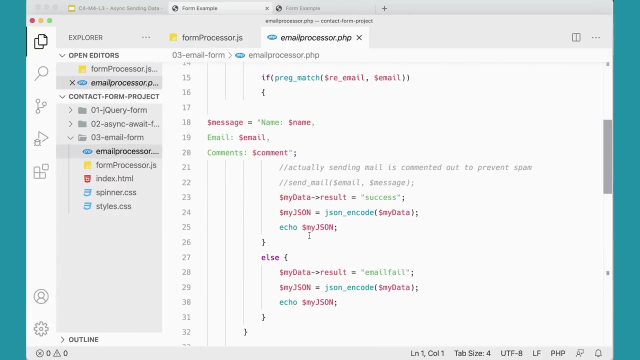 and look in my console, you'll notice I have the word success here And that's because down here in my send data I'm console logging out that data result there. So that's where that success is coming from. It's showing up because the email processor is returning. 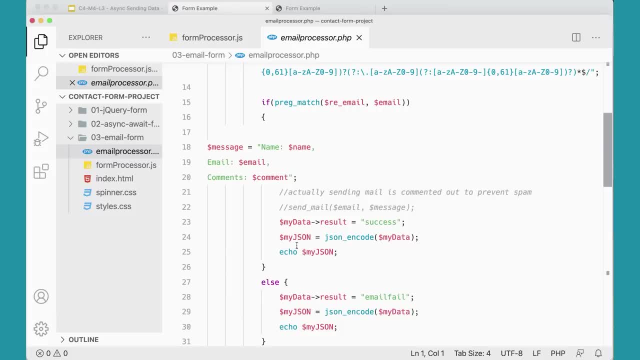 Not only would it actually send the email, but it's actually returning this result. success here. It's not actually sending the email because that's commented out, But there we have it. We have a email form. that is kind of a nice design. 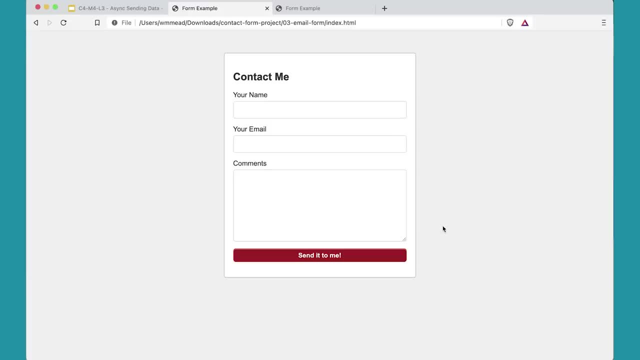 It's got kind of a nice interface, some nice interface elements. It's got some usability features to it. It's something that you could use on your own websites if you wanted to, which is pretty fun. One thing I should mention is that if you're putting it on your own server, 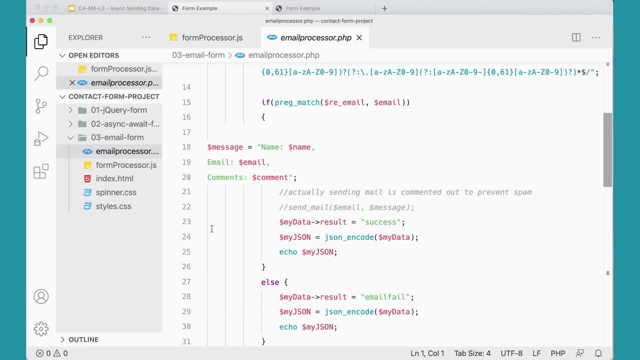 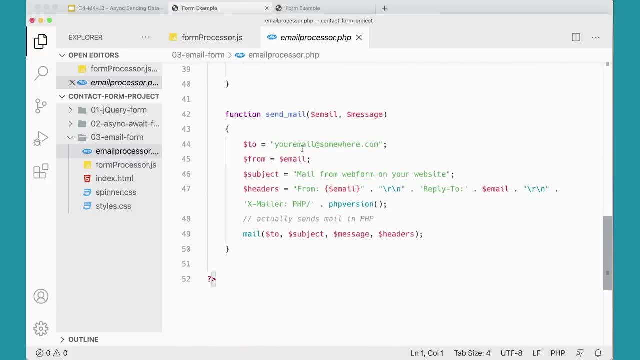 if you're, if you've got, you know, cheap shared hosting on a server somewhere, then on this email form when you put in your email here, like: suppose your website is myawesomesitecom, Generally the cheap shared hosting will only send the email. 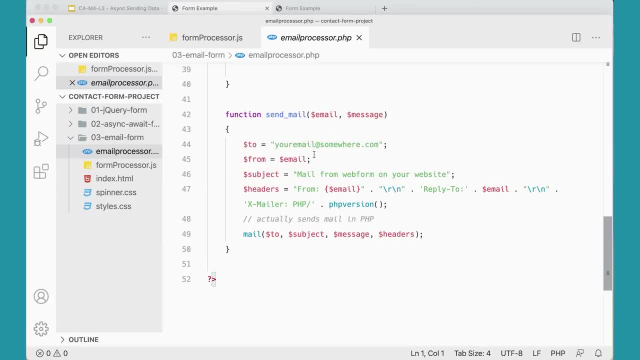 addresses will only allow PHP to send to email addresses within that domain, So you would have to have you know. bob at myawesomewebsitecom is the email address You'd have to be at awesomewebsitecom. 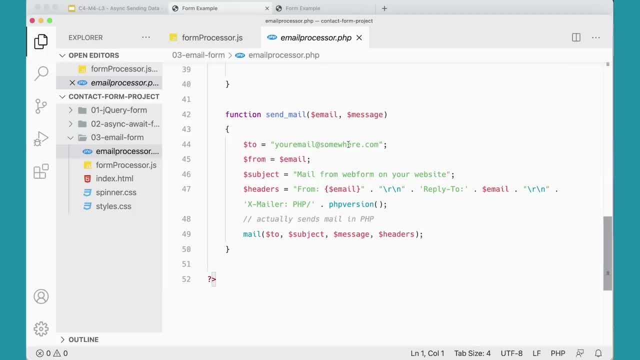 whatever your email address is at that website, You wouldn't be able to, probably, probably wouldn't be able to send this form to, say, your Gmail account or some other email account, just because they, mostly, most of these companies- have, these companies that provide hosting, have their servers locked down in such a. 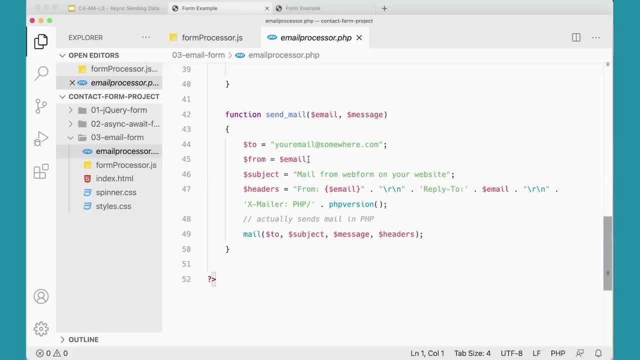 way that it won't allow it to do that, In case somebody hacks into the server. we don't want these servers sending out tons of spam to everybody. all over the world There's a lot of bad actors that are trying to trying to take over servers and do that kind of thing. 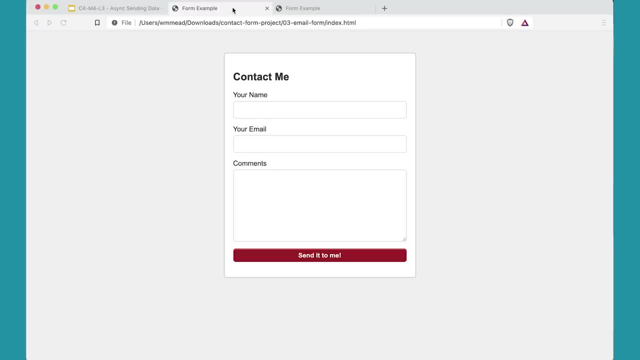 But this is a lot of fun. This is a really great project. I hope you've had fun making it and making all of these projects with me throughout all of these courses, And I hope you find them useful. I've really enjoyed putting them together. 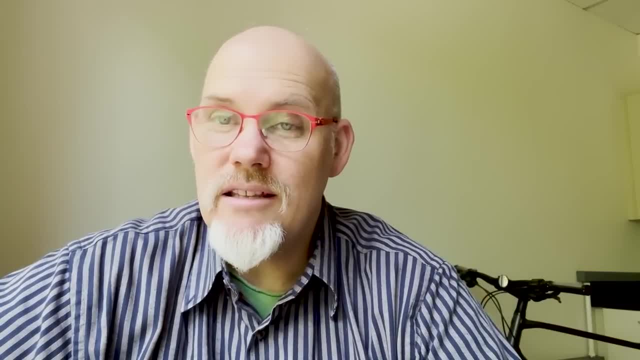 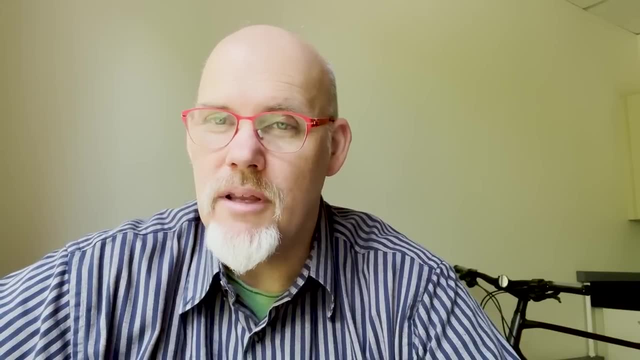 Congratulations. You've made it to the end of our fourth course and to the end of our four course specialization on JavaScript. That's a lot of JavaScript and you've spent a lot of time on this and you should be really proud of yourself In the first course. 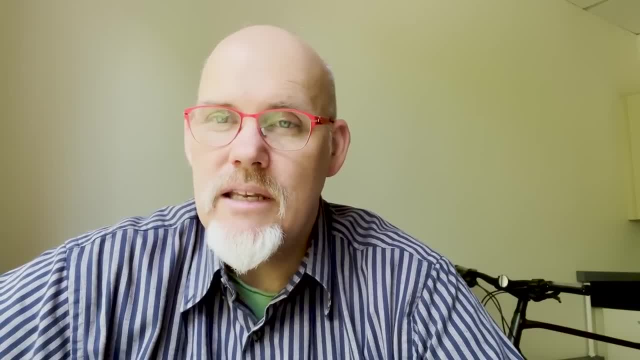 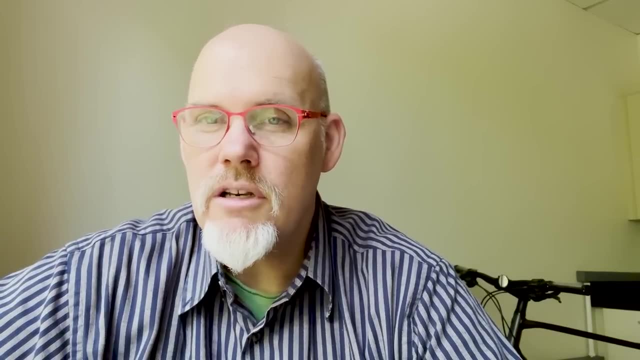 we covered a lot of basics and when you started that course you probably didn't even know that much about JavaScript. But now, if you look at what we've done over these four courses and what you've learned, you've come a long way. 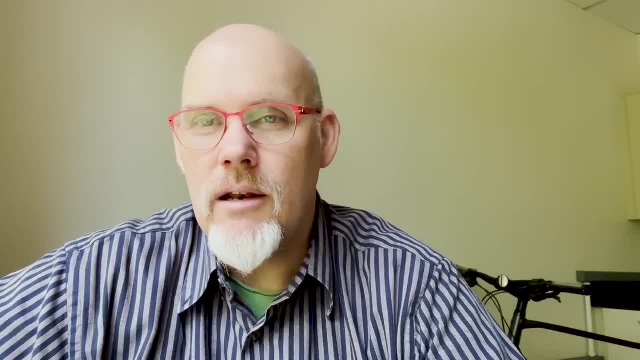 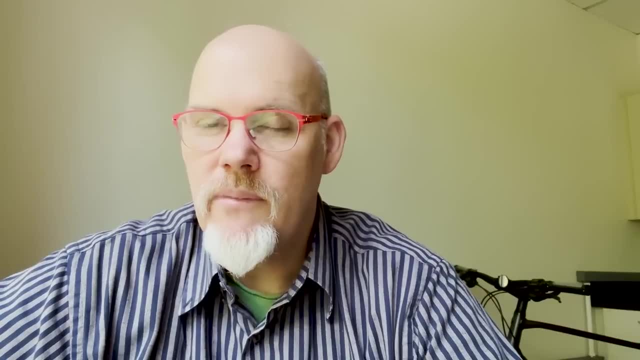 In the second course we got into jQuery and how to create some animations and create some interface elements that we can use on web pages, And that was super fun. In the third and fourth courses we got in even deeper, worked with jQuery plugins. 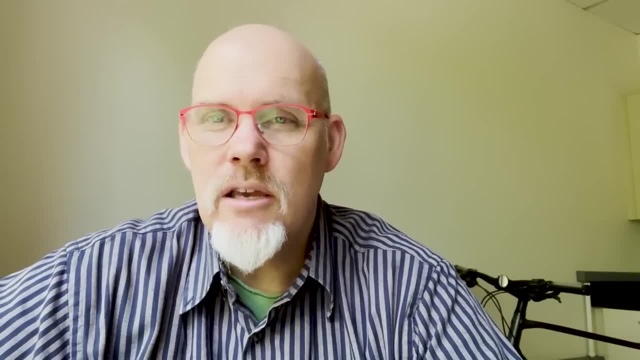 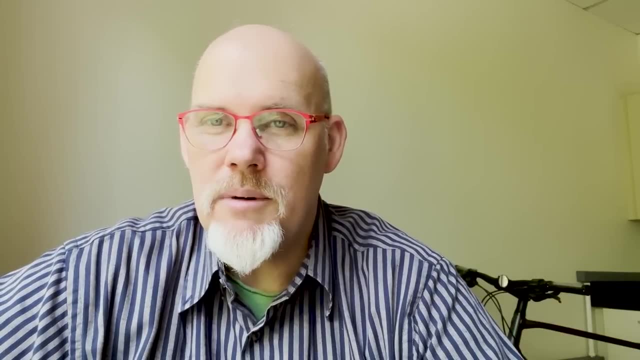 built some JavaScript little web applications. We even got into some asynchronous JavaScript. So that's a lot to do in these four courses and I think you should be really proud for being here and for working through all of that material. I've had a lot of fun putting together that material and I want to thank 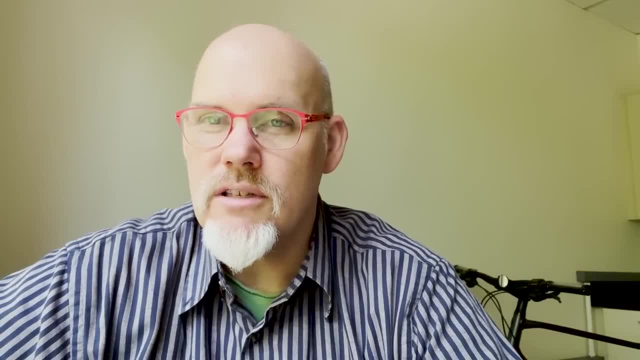 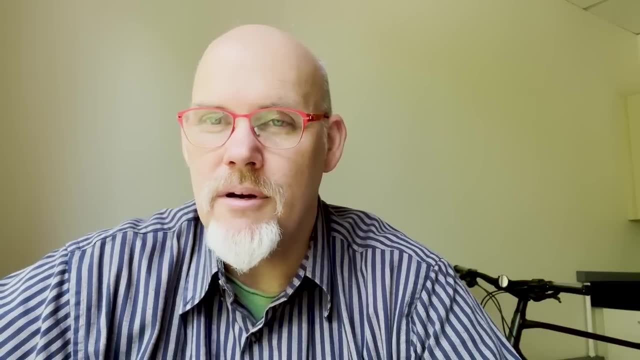 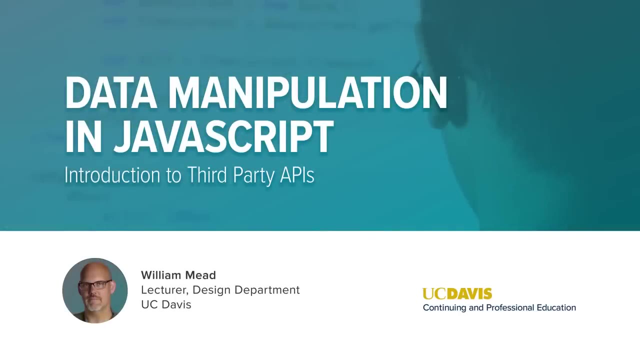 you for sticking with me and working through these four courses. I'm sure that if you keep practicing and keep working on it, you'll continue to progress, to become the kind of developer that you want to be and to meet your goals. Thank you. 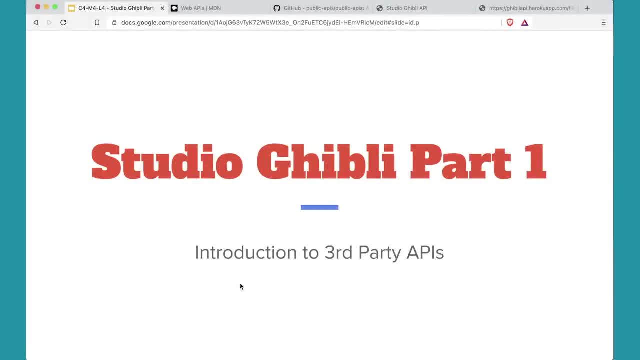 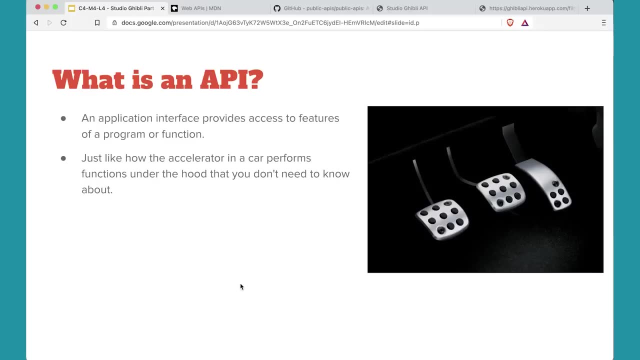 Studio Ghibli, Part 1. Introduction to Third-Party APIs. What is an API? API stands for Application Programming Interface and it provides access to features of a program or a function. Let's take a look at an analogy. When you get in your car, you step on the accelerator and expect the car to go. 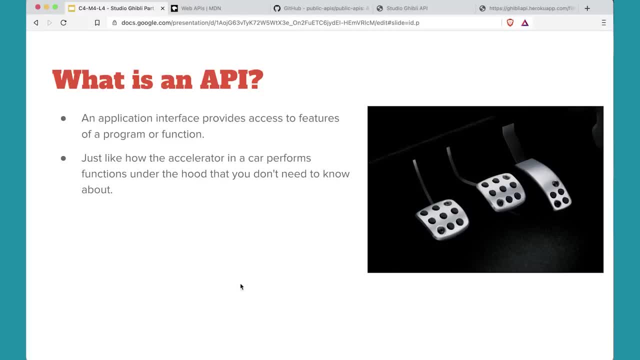 You don't have to think about all the things that are happening under the hood in order to perform this task and interact with the vehicle, And the accelerator pedal is an interface that allows you to do something with your vehicle. Your vehicle has other interfaces. 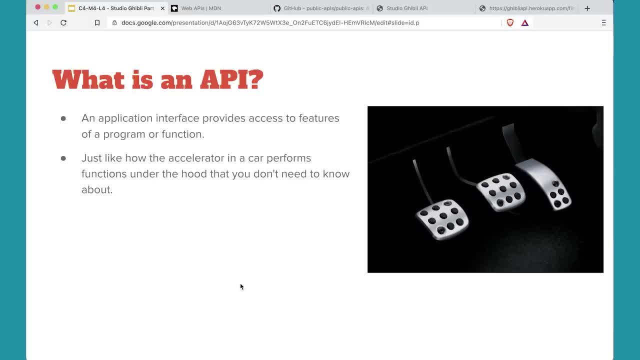 How often do you think about what a transmission actually does? Yet you know how to change gears in your car. These are features of these particular objects that have been designed that allow people to interact with them without having to know what happens under the hood. 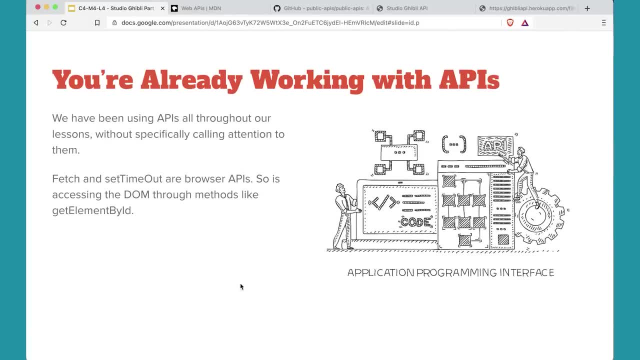 We're already working with APIs, and we've been working with them throughout all of our various lessons, without specifically calling attention to them sometimes. The Fetch API and SetTimeout API- these are all browser APIs, So is accessing the DOM through methods Like getElementById. 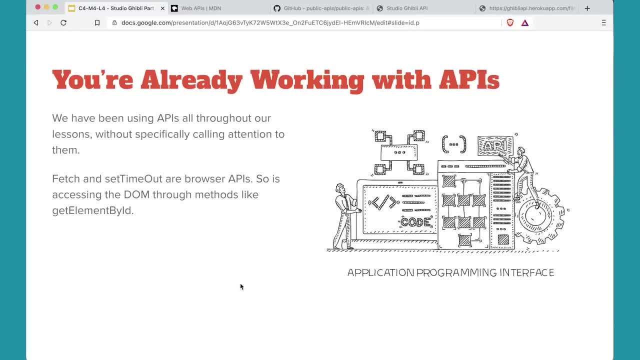 These are all APIs that provide us with ways of working with JavaScript, with browsers, that we don't have to think about the programming behind it that makes the browser actually do stuff. We can just use these functions and these methods that allow us to do things within JavaScript. 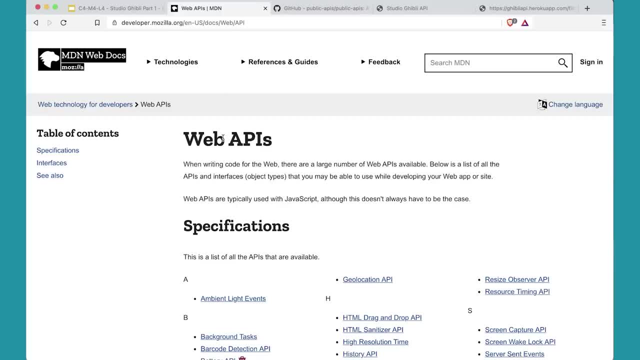 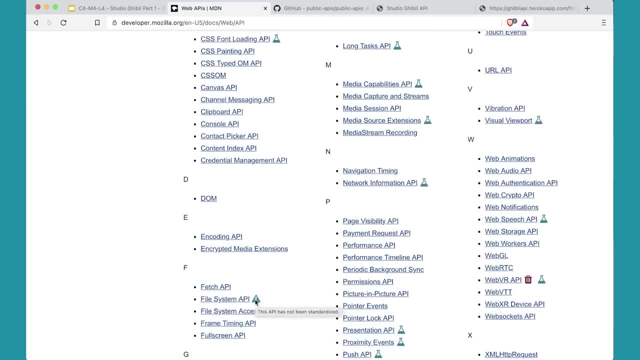 And if you go over to the MDN and look up web APIs, you'll see that there's tons of them, And in this list you'll see the DOM API, Fetch API. Some of them have warnings next to them and some of them are experimental. 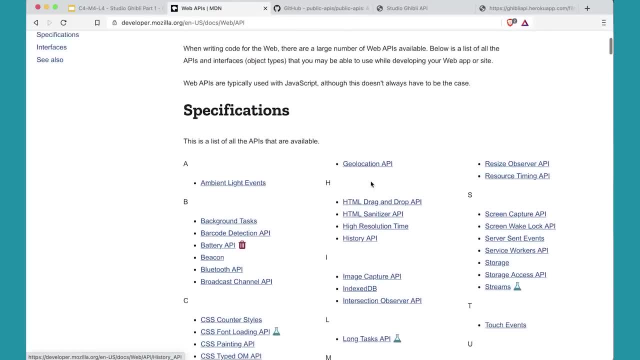 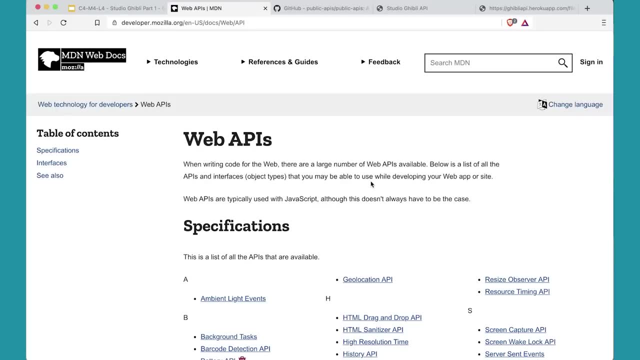 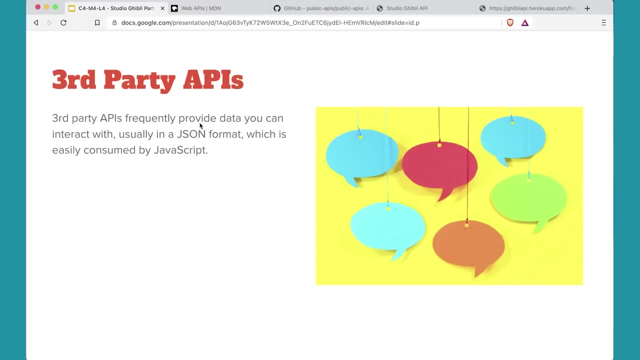 But there's lots of great APIs that are being worked on by people who develop browsers that allow us to do interesting things with JavaScript and browsers, And that's what these APIs are doing here. Third party APIs frequently provide you with data that you can interact with. 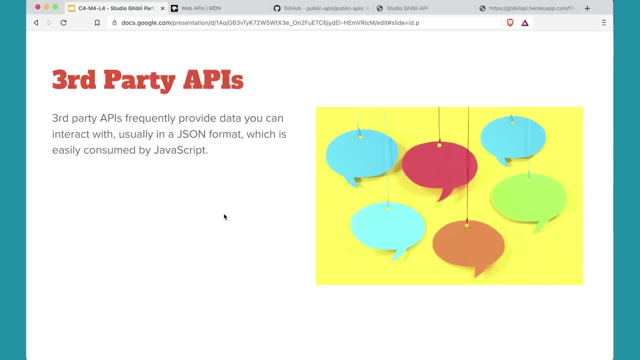 They're usually in JSON format, which is easily consumed by JavaScript, so that's really great, And by working with third party APIs, you can create all kinds of interesting applications. Some APIs require that you sign up and use an API key to access the API. 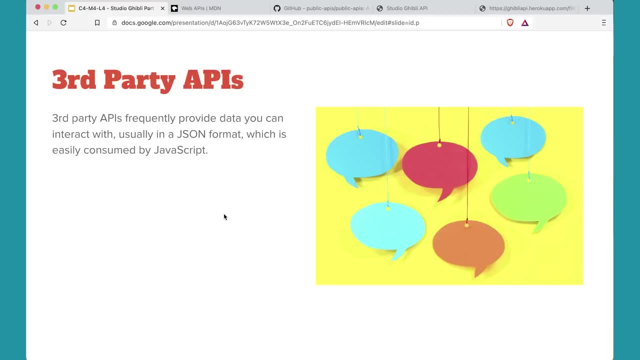 Others allow free access. Some of them will charge you for access if you go over a certain amount of data or a certain amount of hits of the data, So you need to be aware of that. If you're making an application that's going to be popular and used by lots of people, it may end up costing you some money once you hit it a certain number of times. 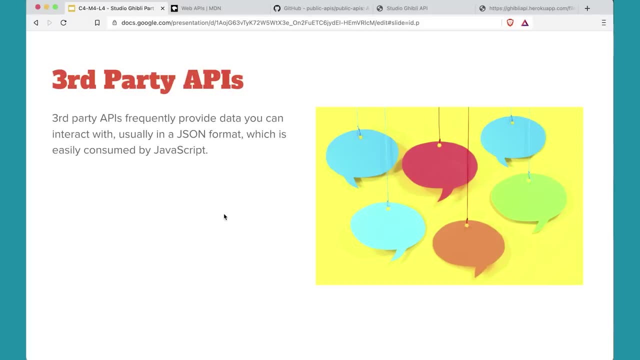 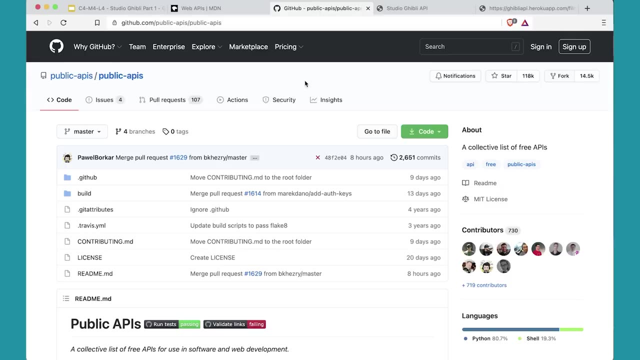 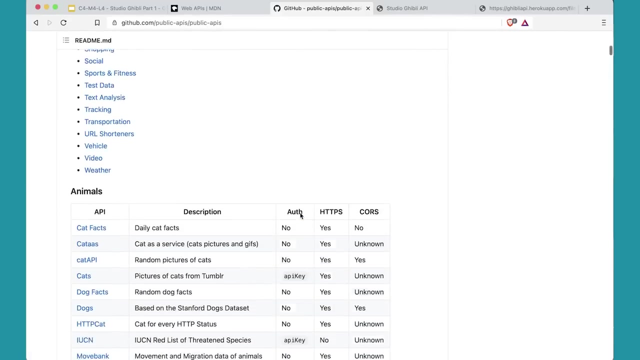 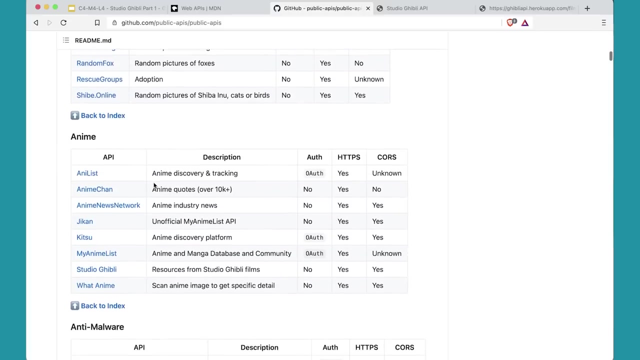 Some of the popular third party APIs include Google Maps or Twitter, But there's a really great list of publicly available APIs out on GitHub And I'll leave this link for you in the lesson as well. If you come through and look here, There's tons of APIs that you can access: information about dog facts and random cats and all kinds of fun useful things, or maybe not so useful things. 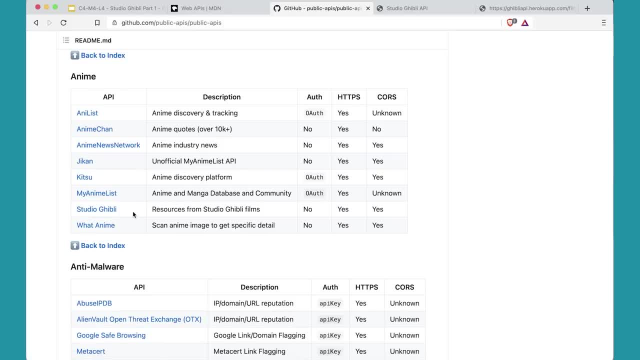 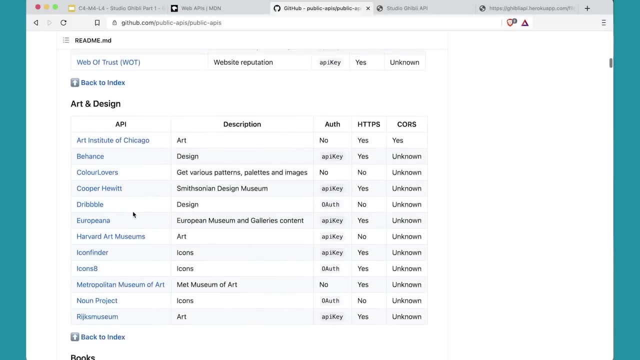 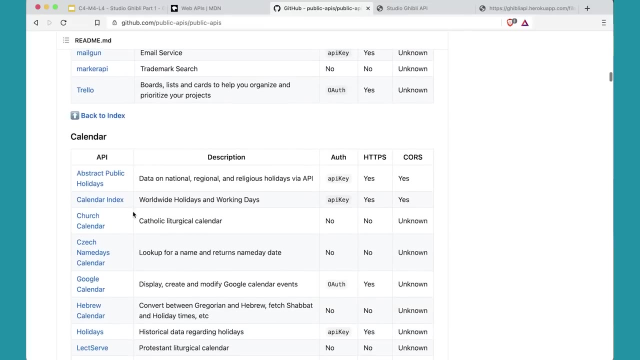 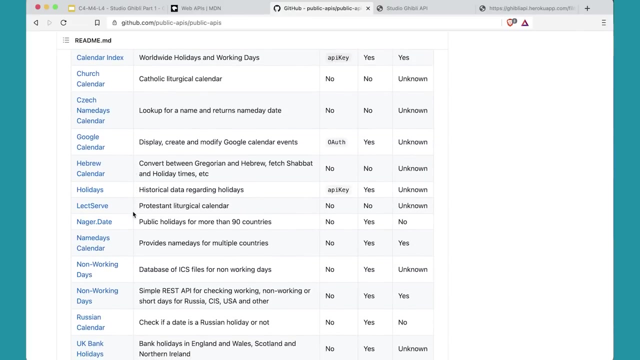 We're going to use the Studio Ghibli API for this particular project, But you could go in and try some of the other APIs if you're interested in seeing what they have to offer. And just like, Just like With the, with the, the plug ins, with jQuery- APIs are being provided by different people and they come with different documentation and you have to really look through all of that. 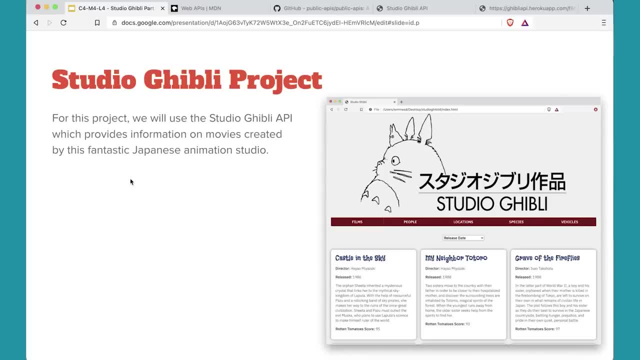 But we'll get to that in a minute. here Again, we're going to create a project using the Studio Ghibli API, which provides information on movies created by this fantastic Japanese animation studio. You can download The start files, which include all the files you need. 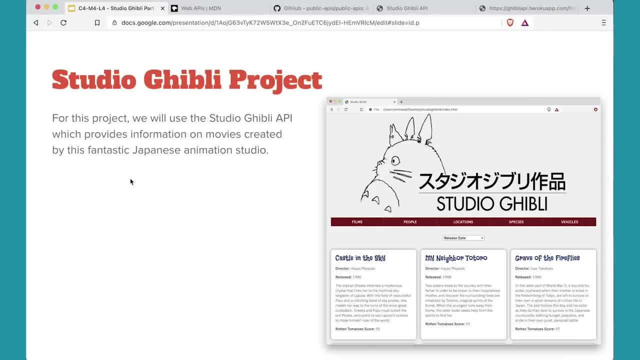 The HTML file has all the HTML file as all the HTML on it that we need to get started. The CSS includes some basic styles and we can add to those a bit more later. The JavaScript file is empty and that's where you'll be doing most of your work, or pretty much all of your work. 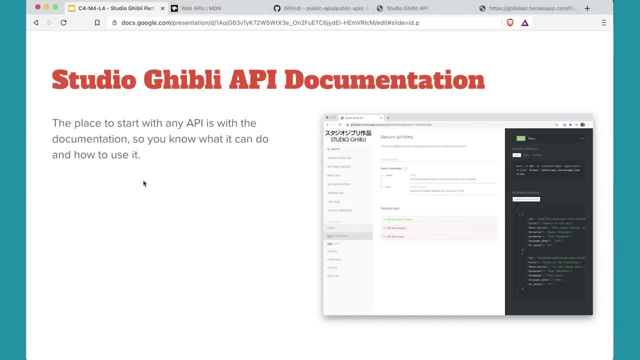 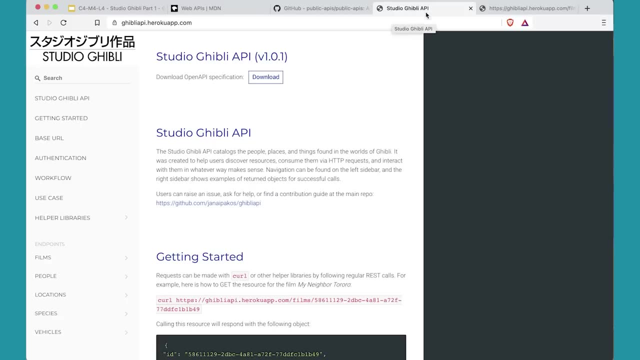 We'll talk about the files in a minute. But the Studio Ghibli API comes with a lot of information. The Studio Ghibli API comes with documentation. I have that linked up here. you just Google Studio Ghibli API, you'll get to it. I'll leave the link in the in the directory as well, in the lesson as well, so you can access it from there. 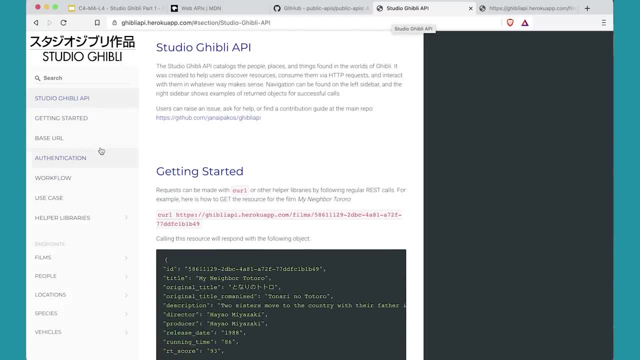 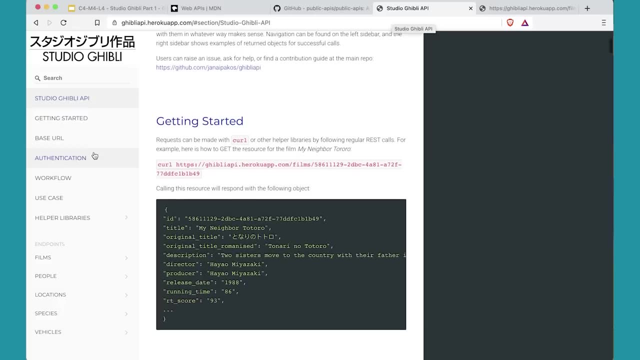 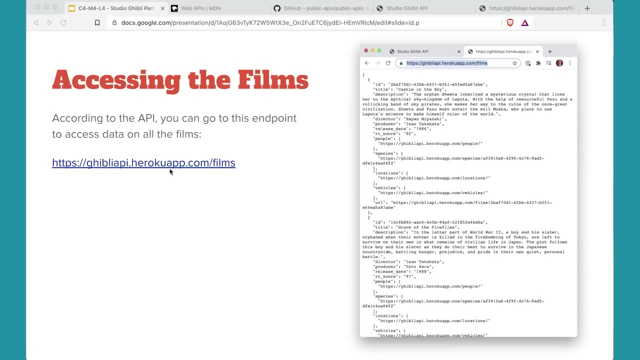 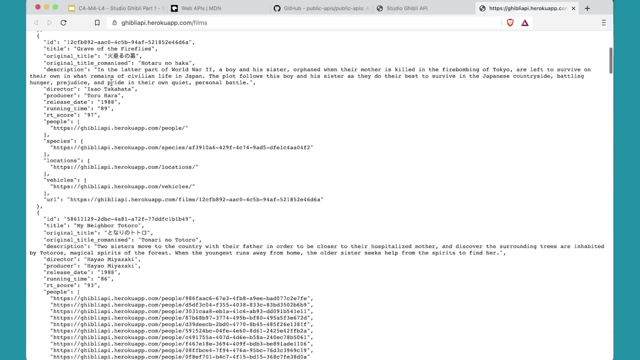 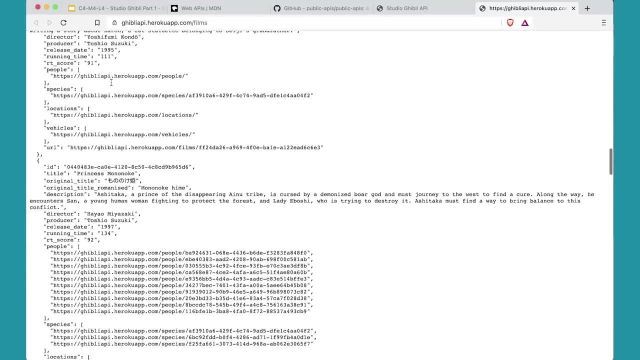 But this, this website, will show you all the directions and give you all the information you need on how to access the data provided by this API, which is pretty exciting. To access the films in the API, you can go to this particular address And I've pulled that up over here and you can see. when you put that in, you just get a pile of data in JSON format, which is exactly what we want, because we can consume this with our JavaScript very nice and easily. 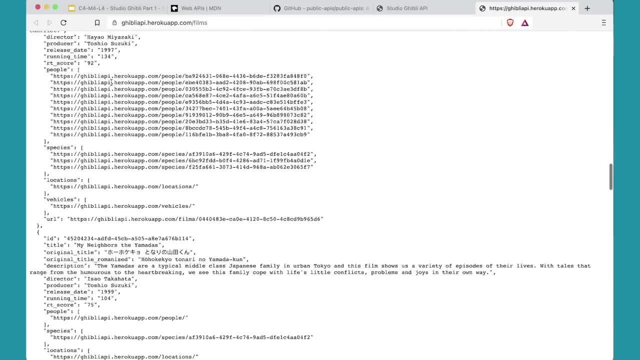 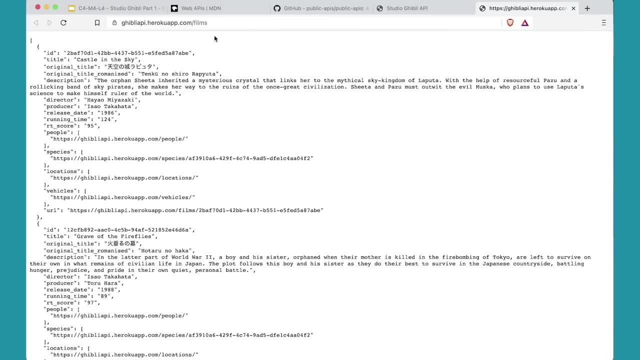 We just get lots of data, lots and lots of data that we can actually do something with, And that's pretty fun and enjoyable, as you'll see in a minute as well, get started on this. so we've got some data, we've got an api to work with, we've got some 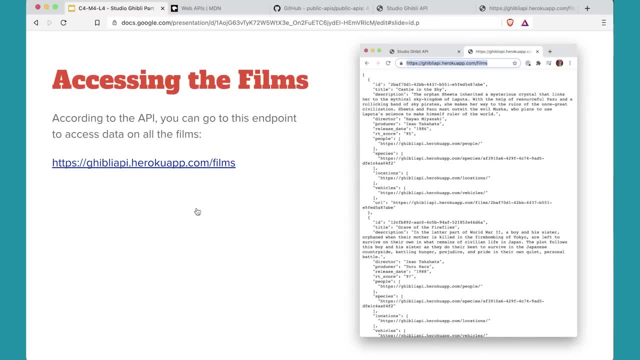 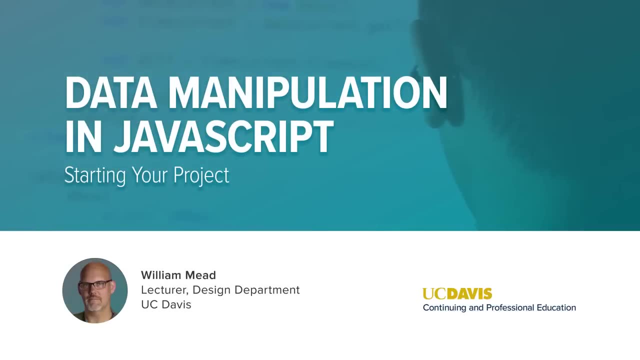 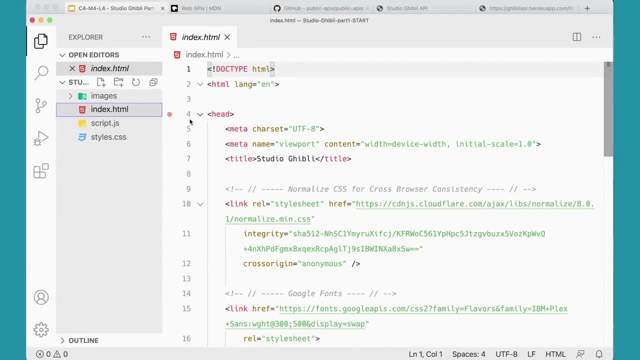 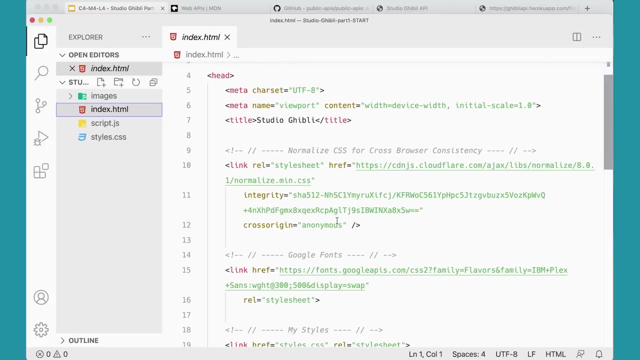 files that we can get started on, and we'll look at those in the next video. download the start files and you can see in here i've got an index file and on the index file i have a normalized script that's just making sure that different browsers are going to render. 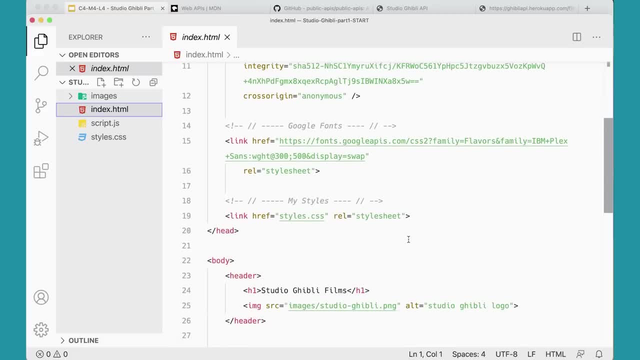 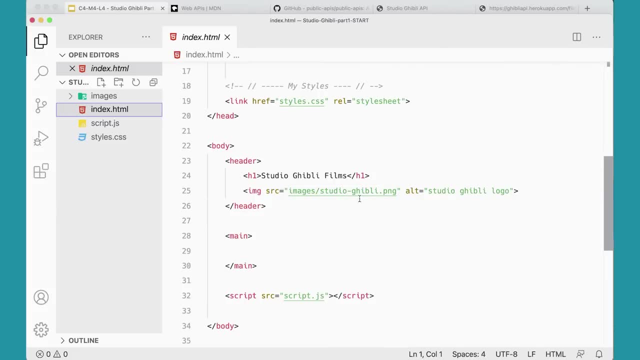 things the same way. i've got some google fonts i'm loading in here, i've got my style sheet and then i have a header with an image. this image is actually simply a picture that i got off of the wikipedia page about studio ghibli films. so that's. that's all there is. i've got a main, empty main element. 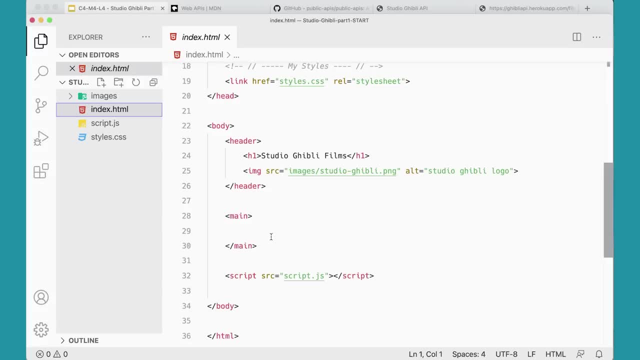 which is javascript, is going to be filling in this element with our movies in just a few minutes here as we get going on this, and i've got a link to a script file which is empty, so we'll be doing a lot of work filling out that script file. the styles are all pretty. 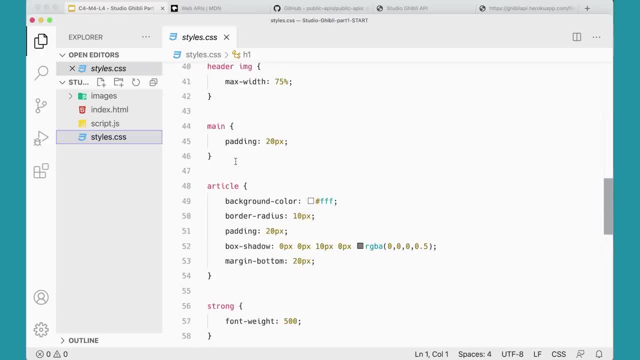 much in place. i've got some basic styling here, not a lot and it's not super huge. you'll notice at the end. i've got some media queries, so this is created mobile first. so i've got a display grid working for tablet size, computer screens and, once you get to 900 pixels wide, for 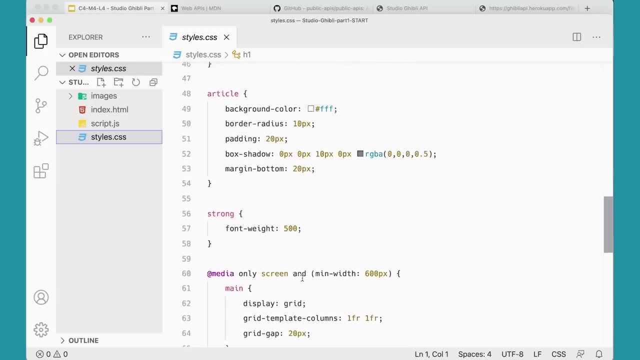 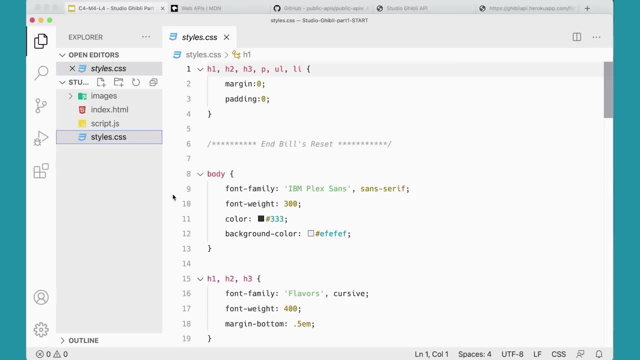 desktop. you've got three columns, so we'll be looking at that here. but but this is all set up so it'll work on your phone and look good on your phone, even with just a few styles, nothing too much, just enough to get us going all right, cool. so what do we need to do? first, let's start by. 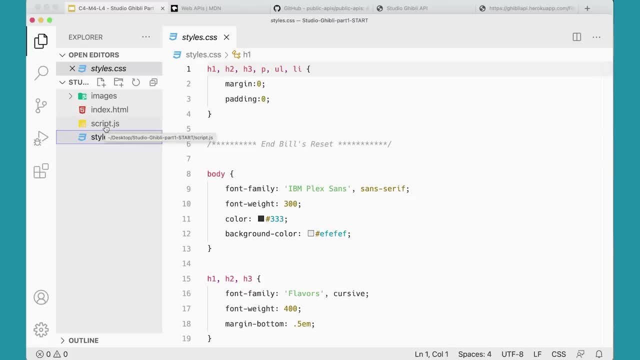 adding some script to see if we can get some good stuff going on here. let's get started with this one. get some data from the API, so I'm going to come over here and if you go to the, let's just go ahead and see what happens. if we add this in here, you're gonna have 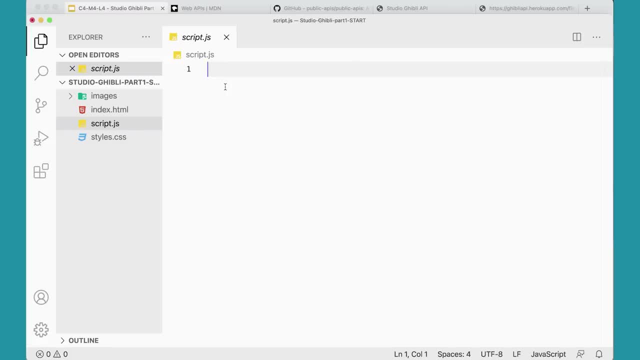 to type it in. I'm going to paste it in. I'm going to paste this in. I've got a variable for my main element, document query selector main. so I'm getting my main element and sticking it in here. we're not going to put anything in there. 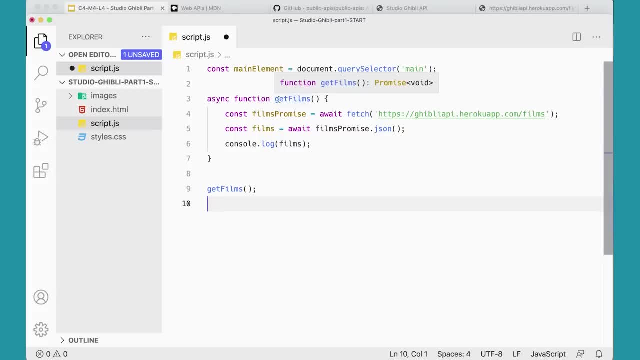 yet. and then I've got an asynchronous function called get films that's going to set up a film's promise and I'm using a weight and I'm going to get that same URL that I put up here initially. so this is just data. we saw that that was just 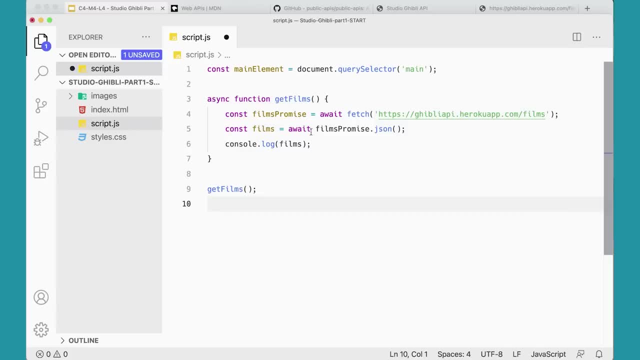 the data that we had before and then I've got a variable films and the weight setting, a weight and price film promise, dot, JSON, because that's JSON data. and then I'm just gonna console log out films and see what happens when I run this get films method here. this: 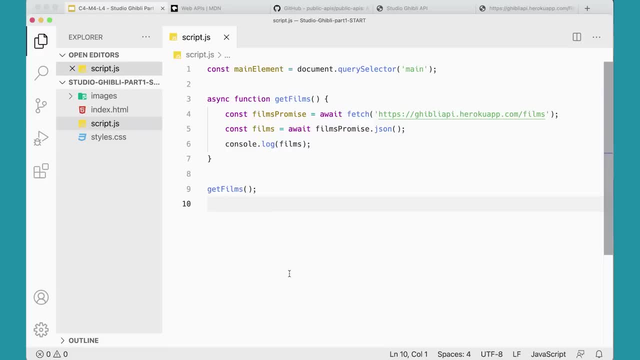 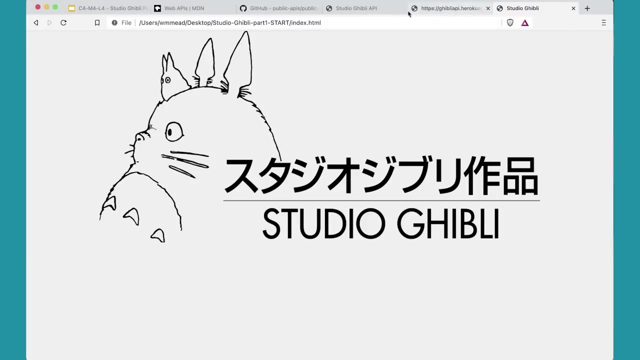 get films function here, so I'm going to save this, and then I need to come over and actually load this up on my screen over here, so I'm gonna I open it up in a new tab over here and I'm going to close out some of these other ones. 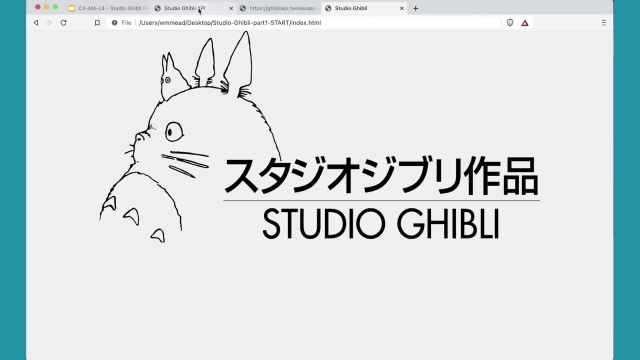 I don't need this one for the moment. this one, the public api's, this Ghibli studio API, could be useful. this one over here. here we go. so the page loaded. did we get our data? let's go in and inspect and click on console and look at that we. 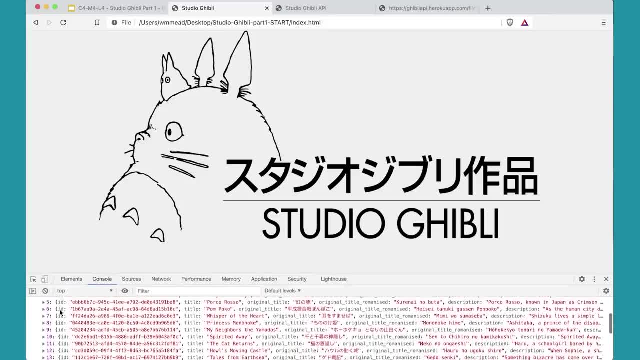 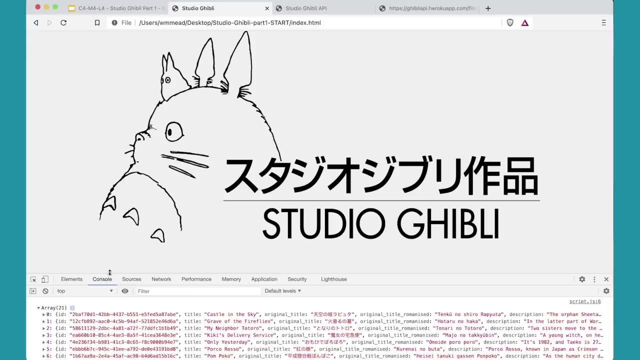 got an array with 21 items in it and if I open that up, I'm getting all of my data. isn't that beautiful? all my data about all my different films. so we're able to get the data coming in to our page really simply using this asynchronous. 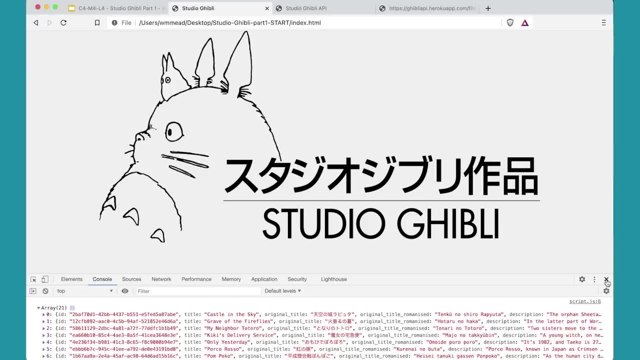 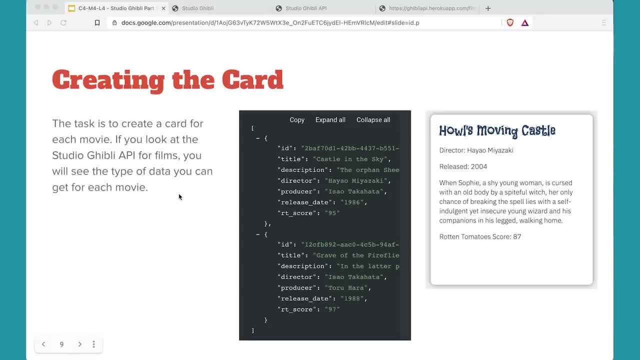 function and that's a really great start. that's exciting. now, if you go back to the documentation for the API and scroll down to the films, you'll see that you can get all of this data for each film, which is really pretty cool, and over here you can see I've got. I want to display that in some sort of card on my. 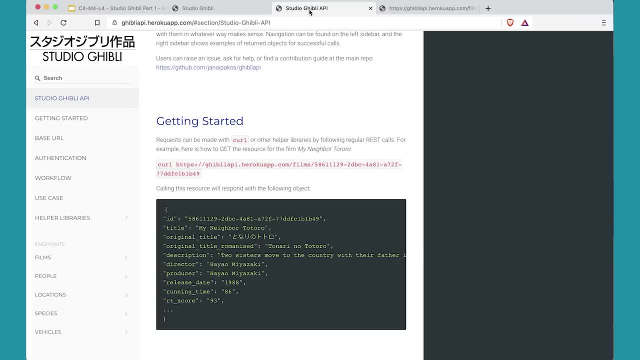 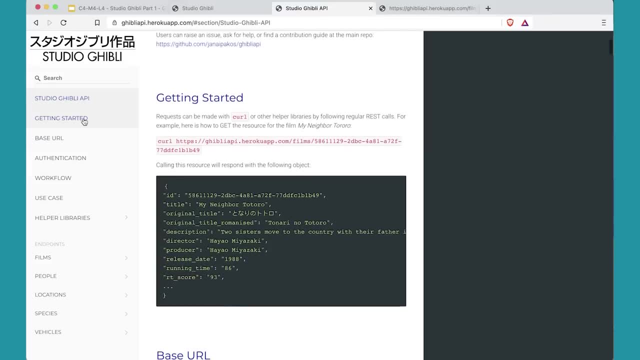 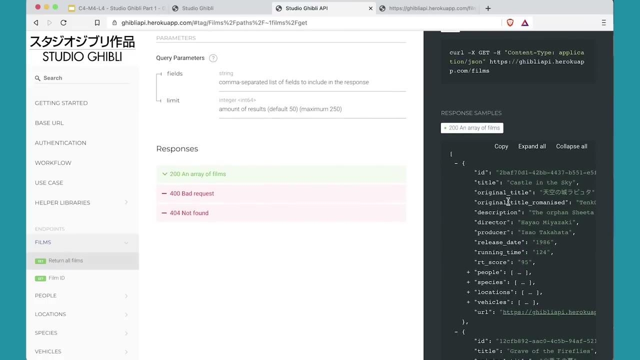 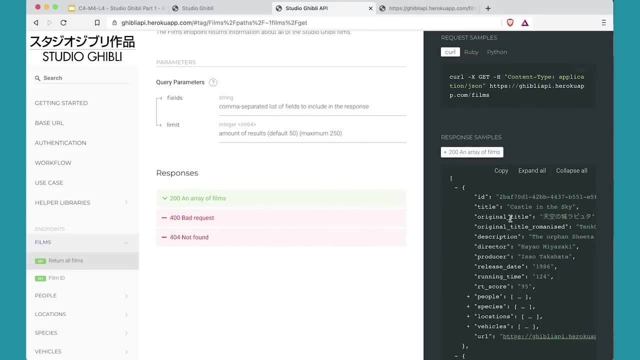 page. so let's go back and look at the Studio Ghibli API here and here. you can see here we're getting some data here. if you scroll down to endpoints films over here, you'll see we're getting all of this data here. thank you that we can get by going to the film's endpoint. 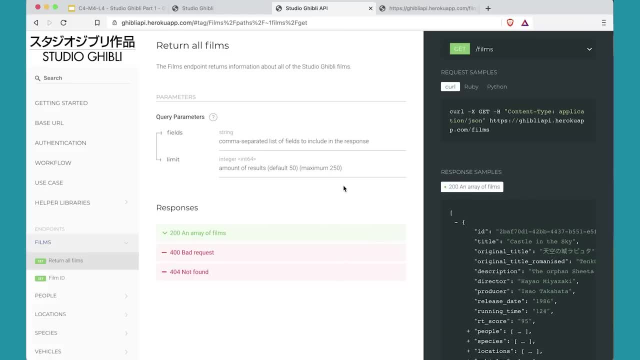 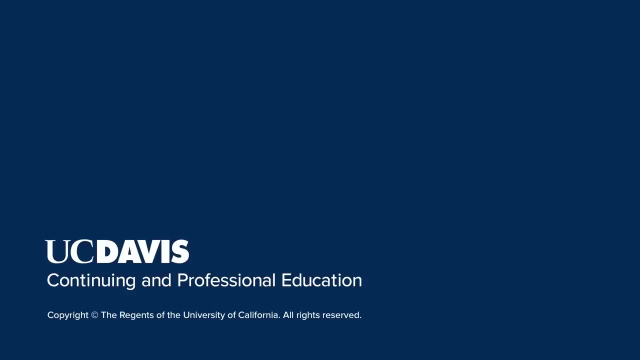 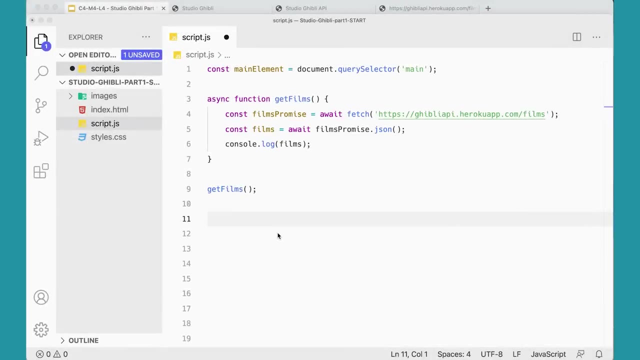 So that's pretty cool. So now we can work with that to see if we can create our card and make that all work. Let's write some. write a function here that has JavaScript. create a card that gets our data from our film's data. 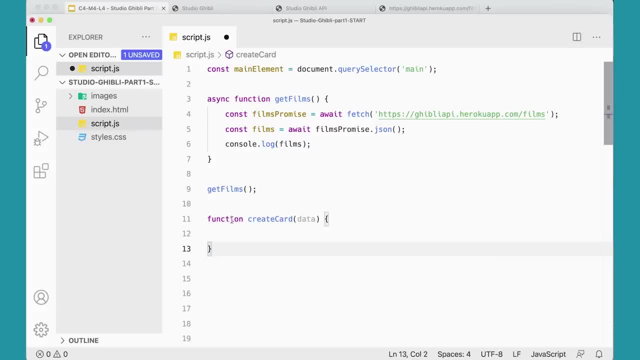 that we're getting here. So I'm going to start by making a simple function Function: create card. I'm going to pass in some data that we'll see how we use that in a minute And then we're going to open that up. 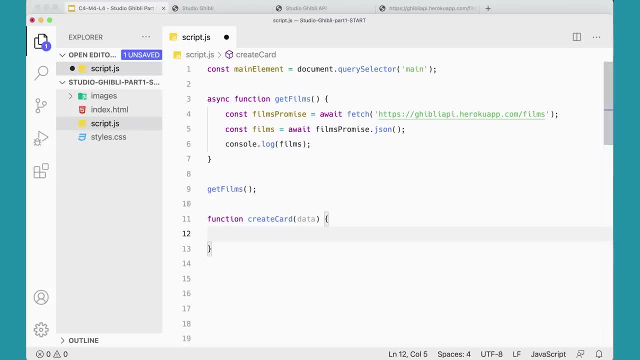 And in here I'm going to create some elements. Start by creating a variable called card, which is going to use the document. create element Articles- that's going to make a new article tag- and stick it into this card variable. just for a moment. 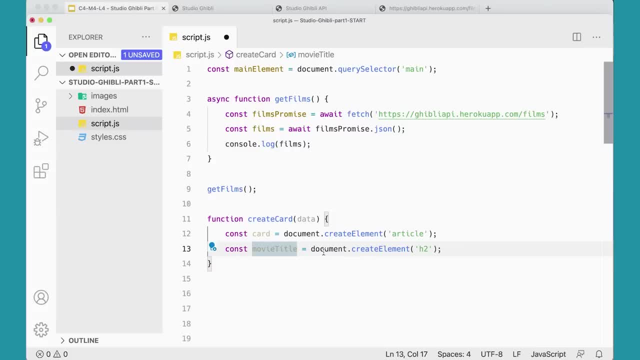 And then I'm also going to make a variable called movie title, which is going to make a new H2 element, and put it into that variable there for a minute. And now I'm going to make a variable called movie title text, which is going to be document. 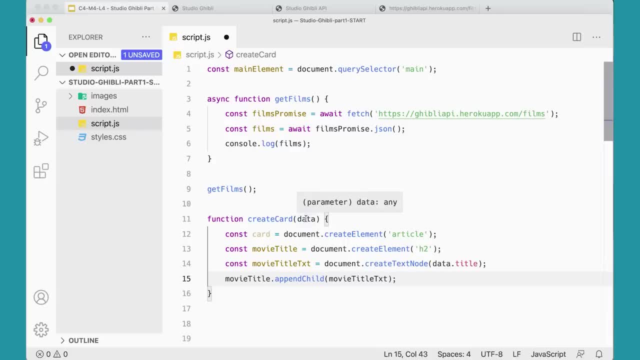 I'm going to create a text node and that's going to get data, this data that gets passed in, But I want the title attribute of that data, the title element in that data, And I'm going to create that text node And then I'm going to take that text node. 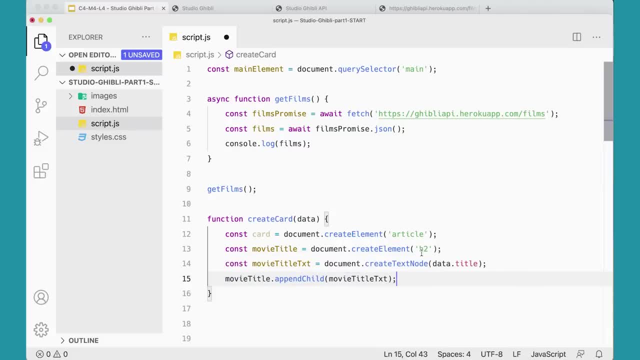 and append it to the title to the H2.. So the H2 will have that text inside of it. Once I have the text inside the H2, I'm going to take the H2 movie title and append it to the card. 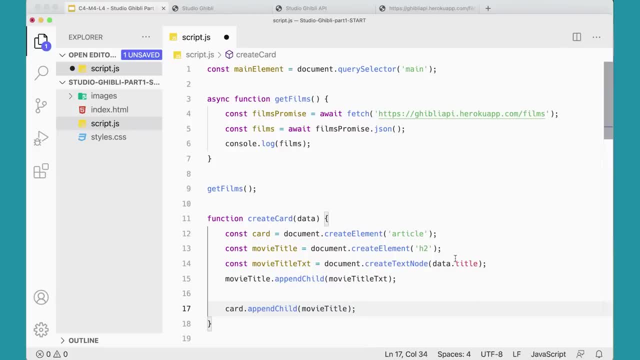 So now the card, the article has the H2, which has the text inside of it, And then, finally, I'm going to take the card and put it inside of the main element. Again, this is our main element up here. 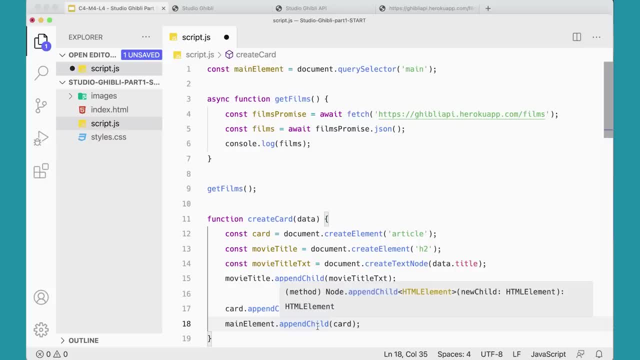 Query, select your main. So we're appending the card to the main element. Cool, All right. So that takes care of. we've created a card, We've created an H2 for the title and we've put the text in the title. 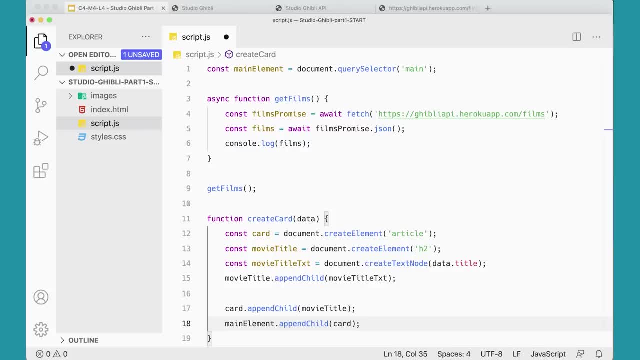 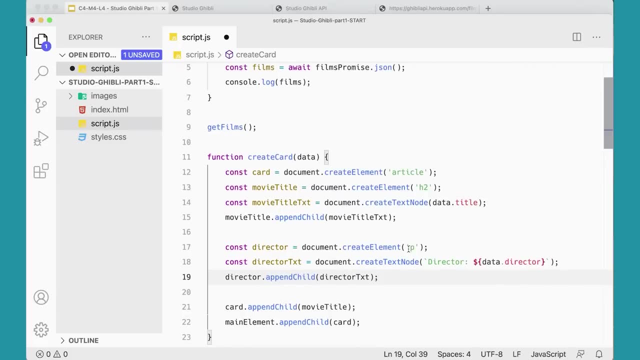 Let's do the next one, which would be the director of the movie, like that. So now I've got a variable director, I'm creating a paragraph, a director text Here you can see I'm using my tick marks to use my template string template thing here. 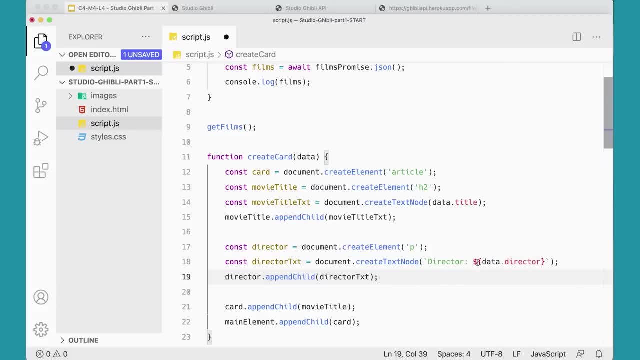 to say director and then datadirector as a variable in here. to get that to display, I'm appending that here And then on the card after the movie title, just copy that one, paste it. And what am I going to append there? 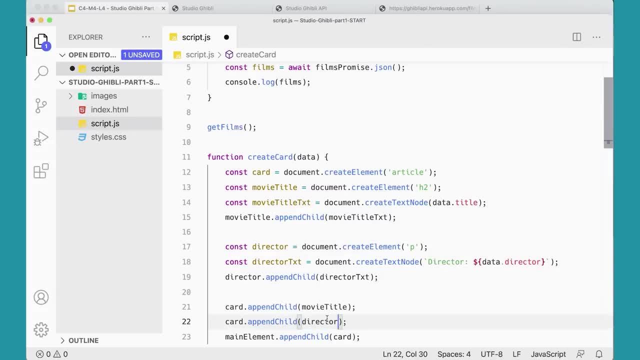 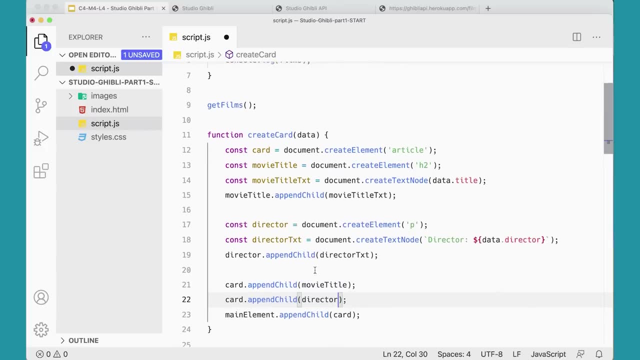 I'm going to append the director Cool, So in this way I can build up all of the content for my individual card that I'm going to use for each of my, for each of my cards, as I go through each movie here. 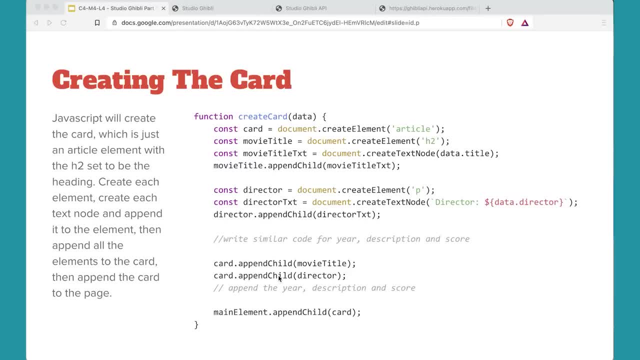 Your job, your challenge, is to fill out the rest of this function. We want similar code as this or this for the year, the description and the score, And then down here, you're going to add those in here as well. You'll append the year, the description, the score. 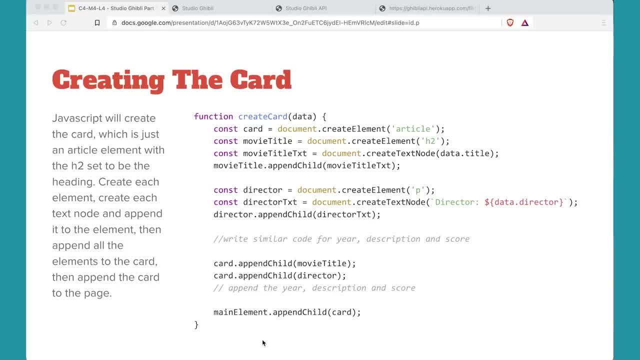 So this is going to get filled out a little bit further down here. See if you can do that on your own And then when we come back in the next video, you'll see how I did it and see if it matches what you did. 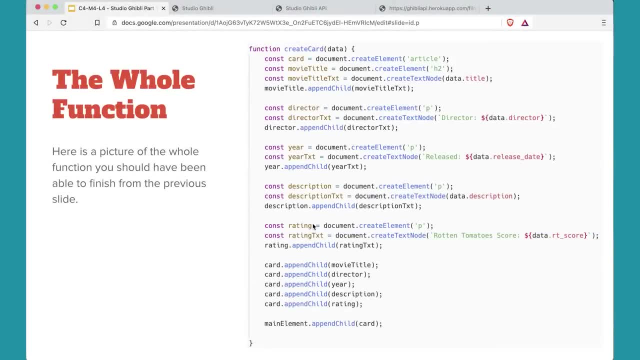 Hopefully you got something like this: If you finish this function, you're going to be able to do the rest of the function properly. So we've got the movie title, the director, the year, the description and the rating, and then we're appending each of these to the card. 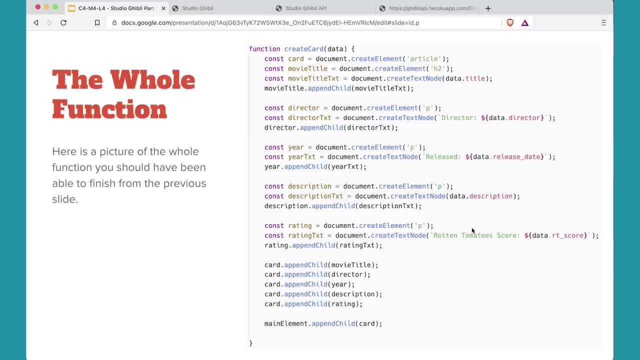 And then we're appending the card to our main element And you can see each one of these is just slightly different. Some of them I have the tick marks, some of them I don't. I'm just putting the data right in the paragraph. 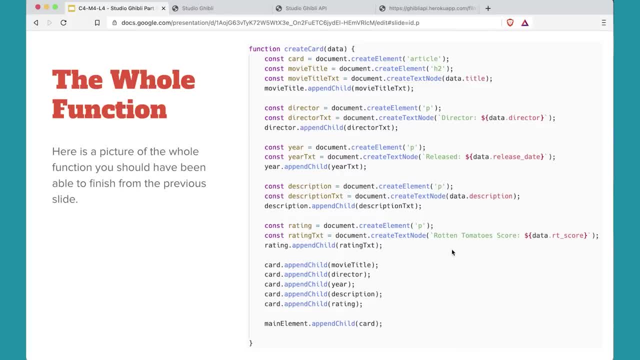 Rotten Tomatoes score, You know, like that, So it depends on what it is, but we're building this up like this, So hopefully you were able to do that. Now your next challenge is to recognize that what's coming through our getFilms function currently. 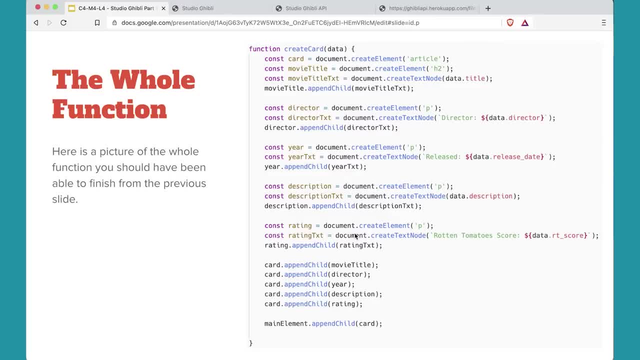 what we're getting is an array of data. Can you use the forEach method to loop through each film and then run createCard on it, And can you do that without going forward in this video to look at the answer? So pause the video and see if you can do that. 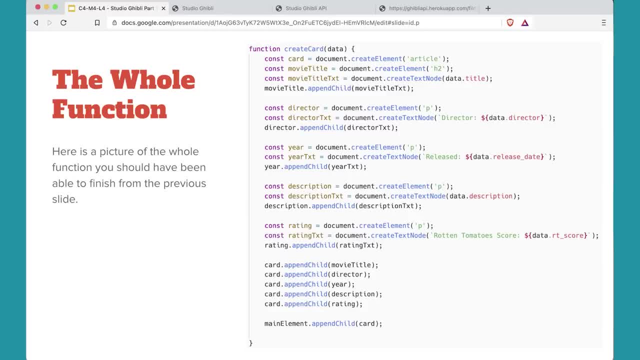 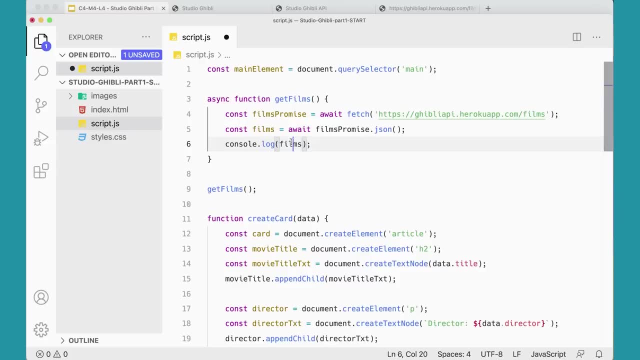 Again. I'm going to sort of specify this even more clearly by looking at the code here Up here. if you look at this, getFilms function here, this thing, consolelog films, this films thing- here is an array, So how could you now use that array to look at the answer? 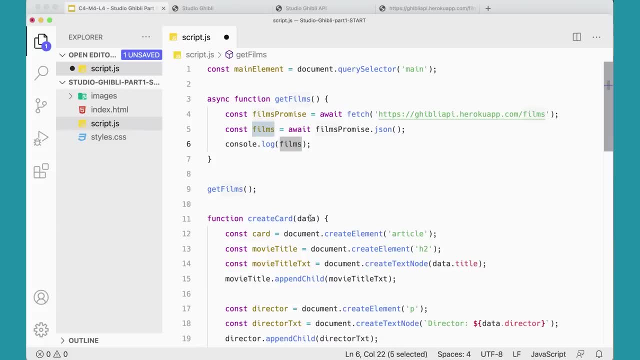 I'm going to use that array with this createCard thing to create all of our cards and get them to display on the page. See if you can do that. Pause the video now And when we come back I'll show you how I did it. 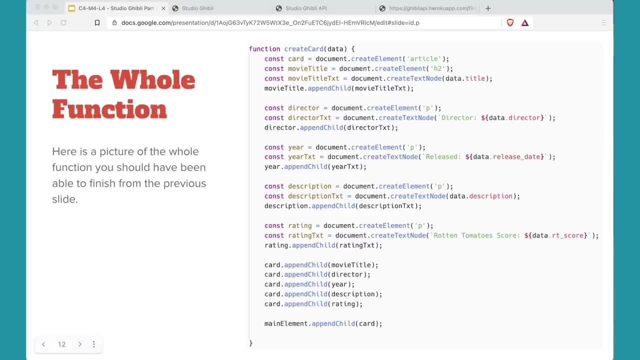 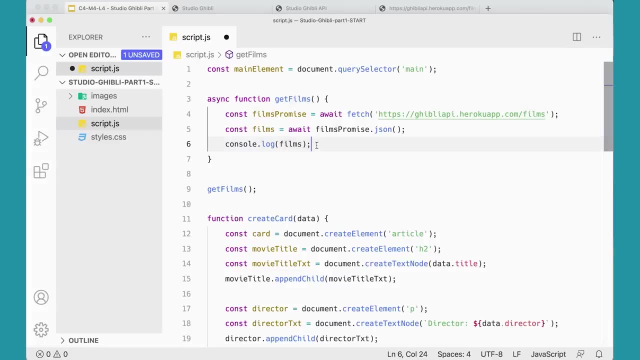 Were you successful, Were you able to do it. This is what I did. I come over here and, instead of just console logging out films, I'm going to run a getFilms function And I'm going to run a getFilms function. 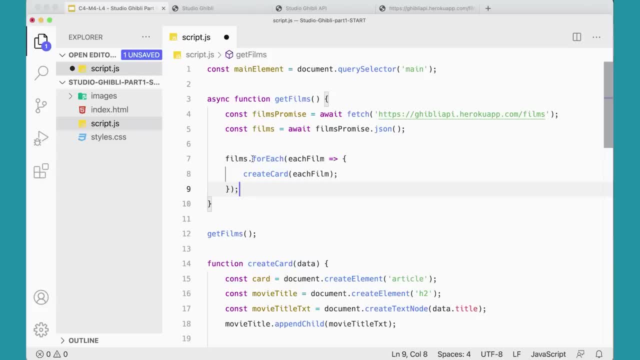 Get rid of that. I'm going to run a forEach loop here, a forEach method, on this films array, And I'm using my arrow function and then I'm running createCard, each film. So this goes through each one of the elements in the array. 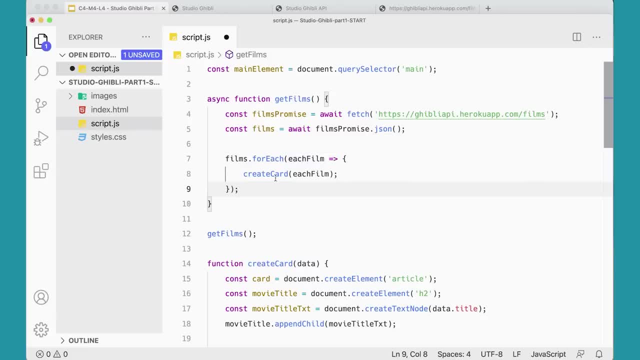 and each one, each film becomes a film in the from the array and then I'm running createCard on it And createCard will take each film and then do all of this stuff to create the card and add it to the DOM. 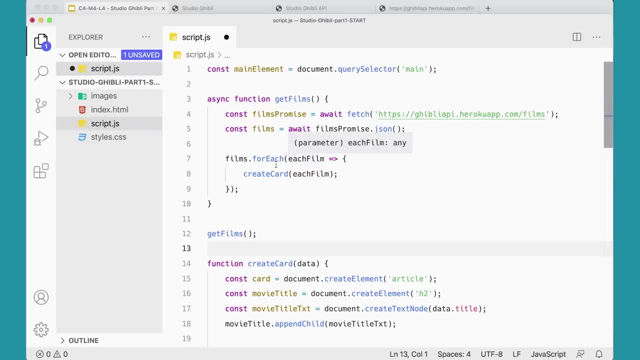 You could have done this with a for loop. You could have done this with a for of loop. There are lots of ways of doing this, but you need some sort of loop to loop through this array to get each film in there. So let's take a look and see if this worked. 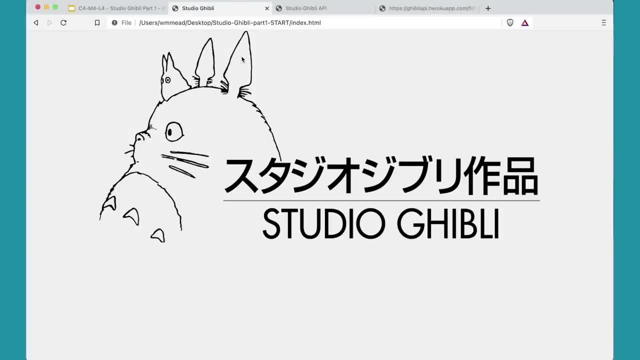 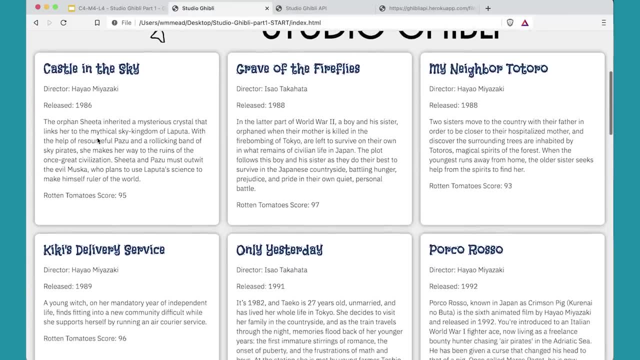 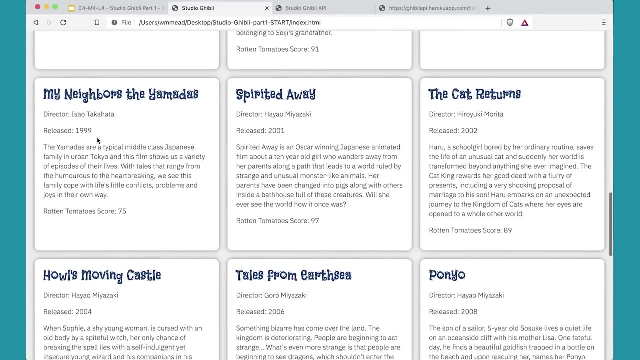 It should have. Let's come over here to our page. If I refresh, I'm now getting films on my page And they look. it looks kind of nice And that's because the styling is already in the style sheet. I've already got this set up to display as a grid. 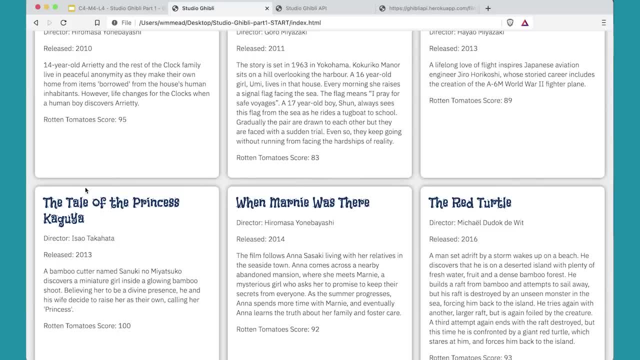 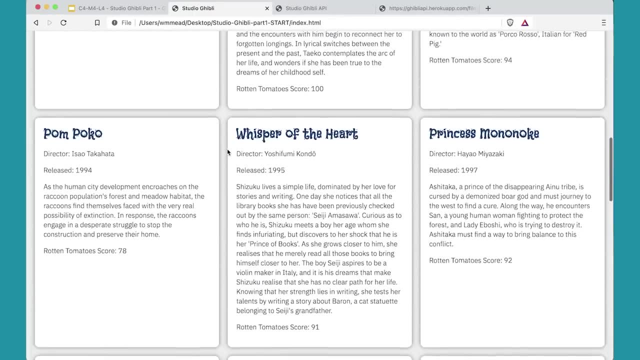 and we're creating our cards and I've got some nice little rounded corners and some shadows here and some typography so that it it looks kind of nice. That's the idea anyway. We're getting our data in there So cool. That's working really nicely. 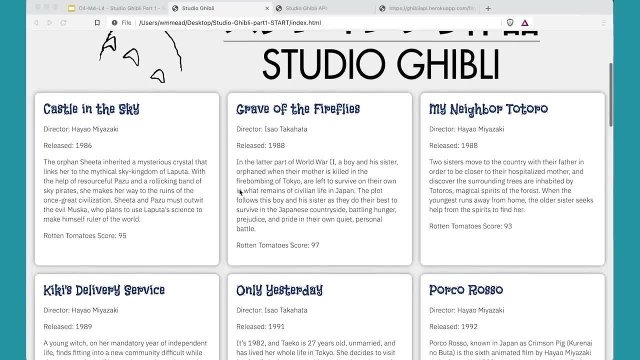 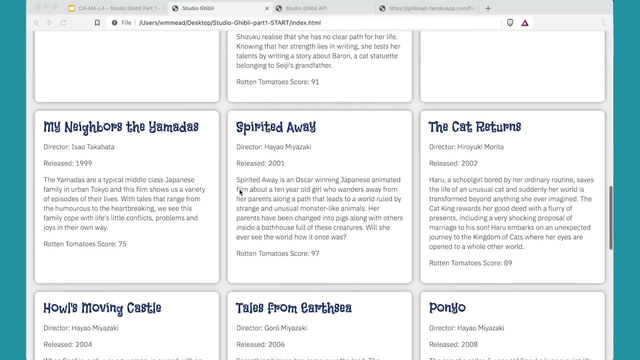 The next thing you might notice is that the films are in kind of a weird order. What is the order of this? It doesn't really make sense. They're, you know, they're kind of just all over the place. It doesn't seem to be in any particular order of any sort at all. 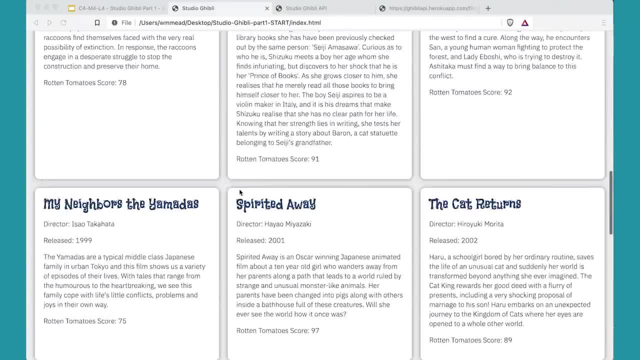 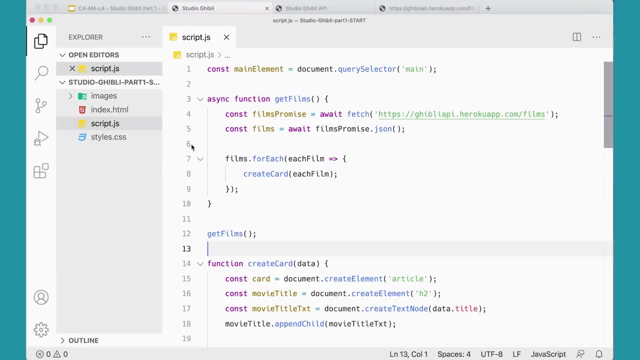 So let's do something to order these films. What I'm going to do is I'm going to come over to my code over here And, before this runs, I'm just going to add in here a line of code. I'm going to paste it in, but you're going to have to type it here, like that. 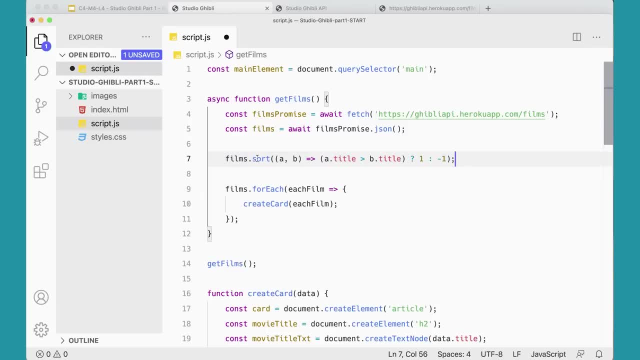 Now here, because films is an array. we're running the sort method on the array And you can go look up that on the MDN. We've looked at that before. But what we haven't done before is pass in a function that will. you can not just sort an array. 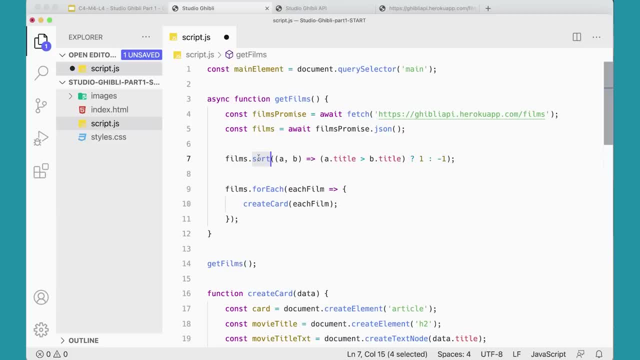 but you can actually pass in a function that will allow you to sort it by a particular field, Like I want to sort it by the title specifically. So you can see I'm passing in a function here And then you'll also notice the ternary operator. 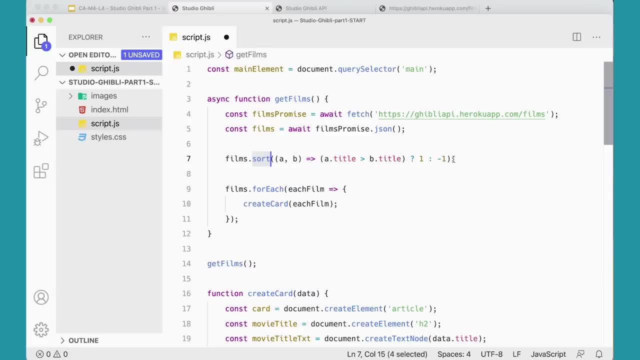 This is not the easiest line of code to read, but it's nice and compact And once you get used to it it's not so bad. But one thing you can do with the sort function is you can pass in an anonymous function. 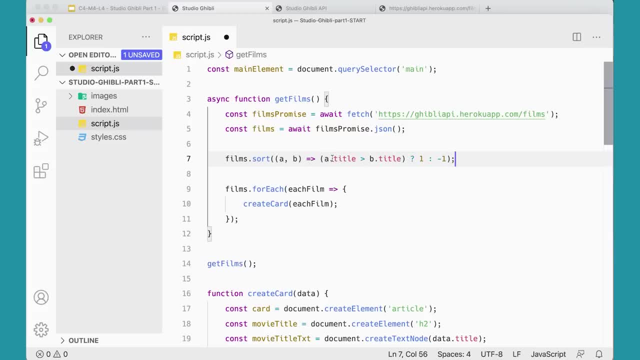 which we're doing here, And you can compare each element in the array to the next element in the array. So I'm taking the first element, A- its title, and comparing it to B's title. If A is greater than B, then this is true. 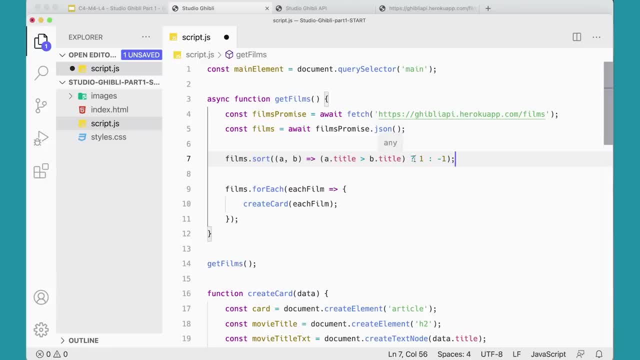 I'm going to set. I'm going to give it a one. If it's not true, I'm going to give it a minus one. So that will move it up if that's true or move it down if it's false. 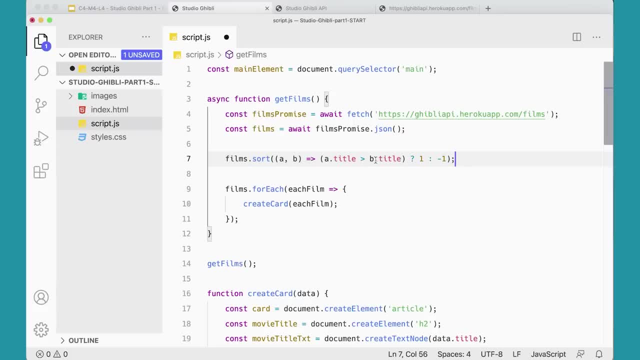 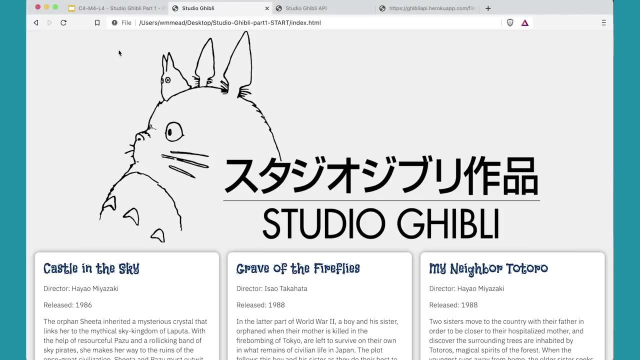 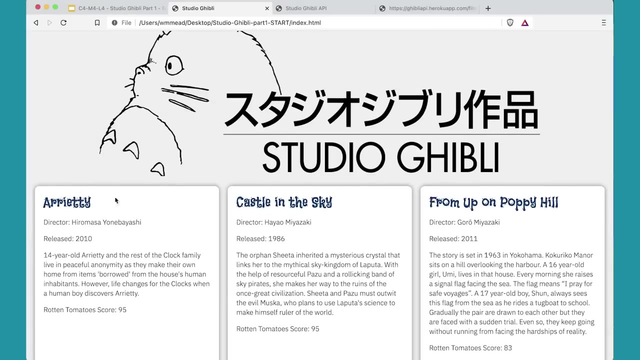 And then these films will get sorted alphabetically by the title, which is pretty nifty. So let's save that and come back over here and refresh the page And look at that. They're alphabetical: A, C, F, all the way down the page here. 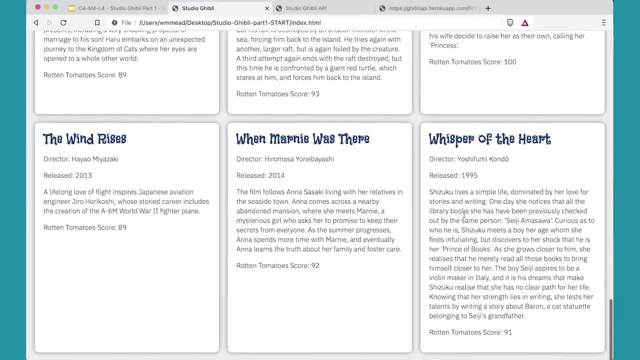 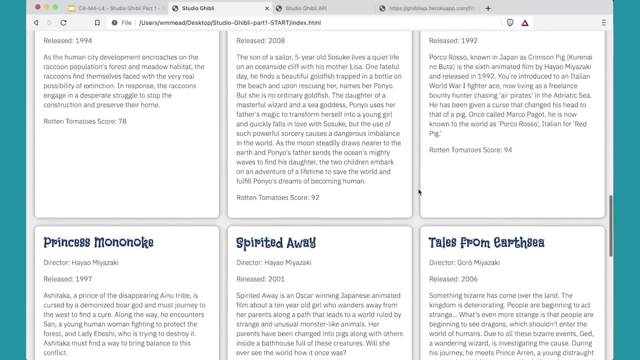 when we get to the end. The last one's a W. You'll notice it took a minute for it to refresh the page And don't forget we're using asynchronous functions, so it might take a minute for you to actually get to the API. 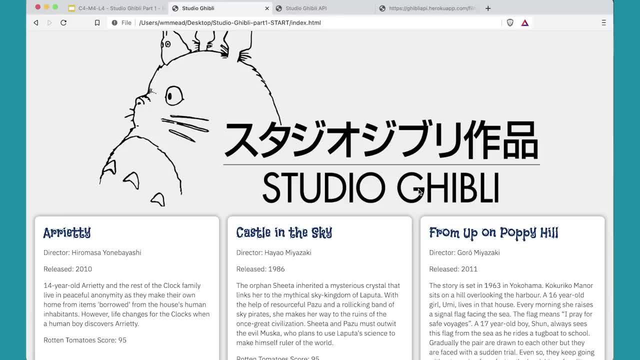 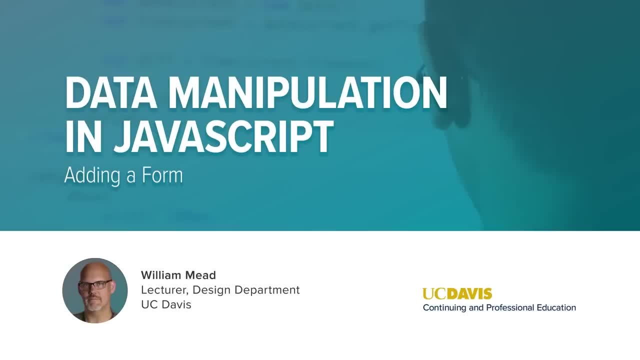 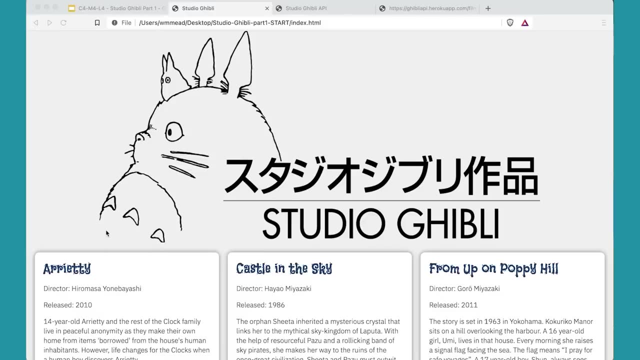 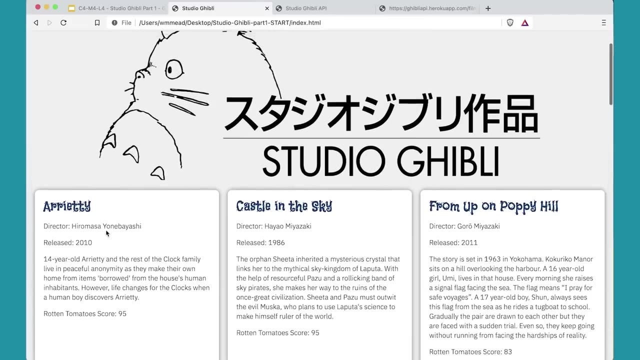 and get all the data, in which case the page will have to wait until it gets there. In the previous video we sorted our films alphabetically, And that's great. So now they're not showing up in some random order. But what if we want to sort in some different ways? 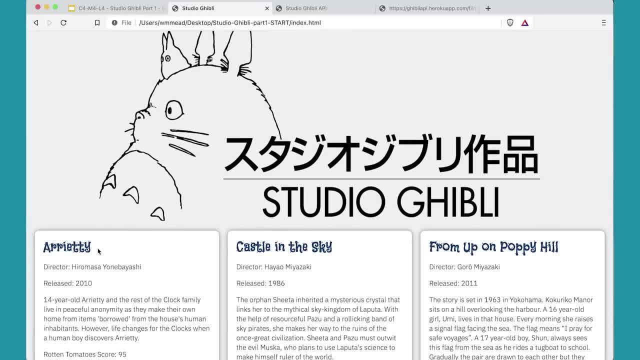 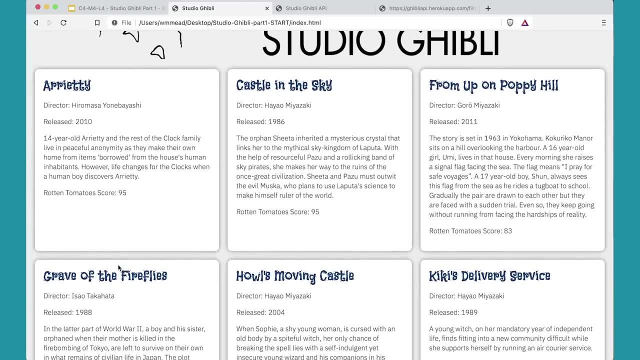 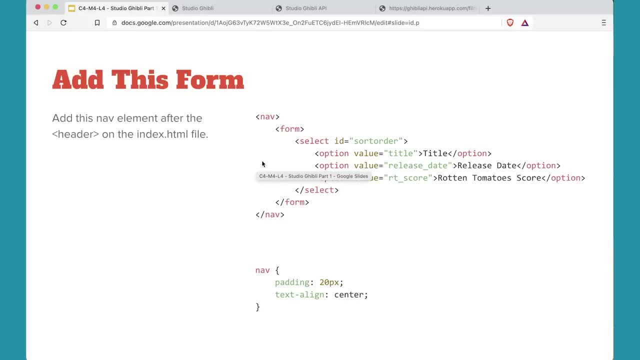 What if we wanted to sort, maybe alphabetically, maybe by when they're released or what their rating is? You might want to see the films in some different orders, So let's do that really quickly. What we need to do first is add some HTML to our page. 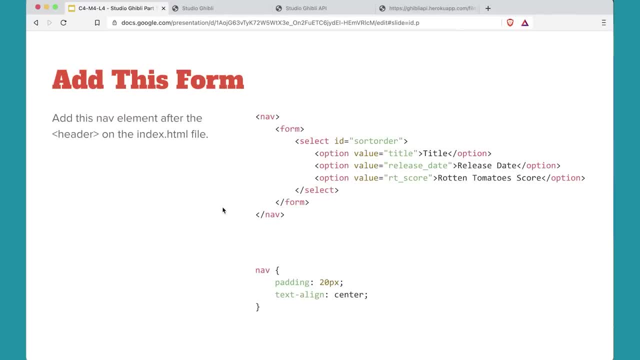 So I've got this- Whoops, I've got this navigation here that we need to add to the page. So let's go ahead and add that to our HTML file, And then we're going to add a little bit of CSS just to center it on the page as well. 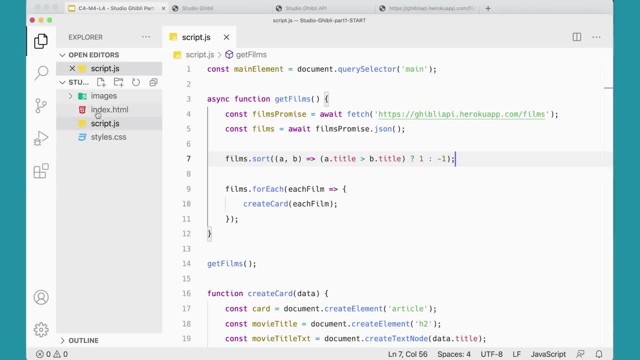 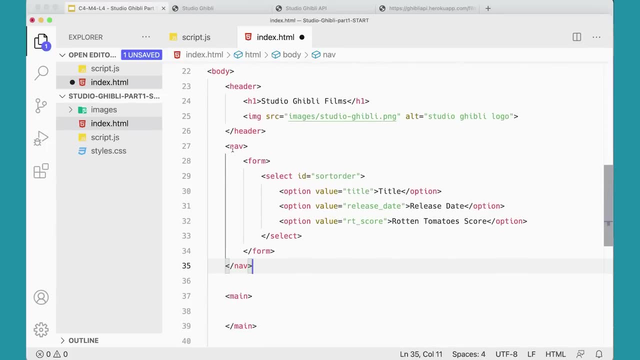 Come back to our code And I'm going to go to my index file And just after the header I'm going to add this nav element. I'm pasting it in here but you're going to have to type it. But there's not that much to it. 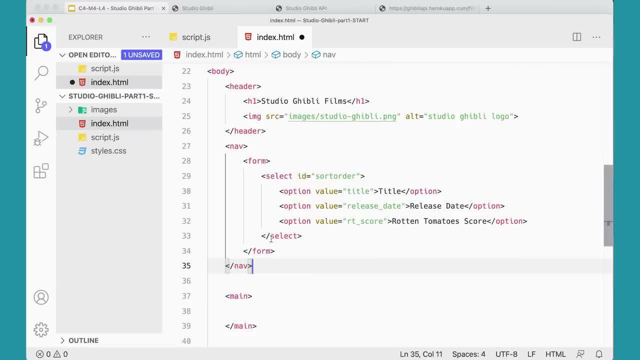 It's just an open and closed nav with a form in it and a select list with some options. Title, release date, Rotten Tomatoes score- just three options, Not too big a deal. It shouldn't take you more than 30 seconds to add this to your file. 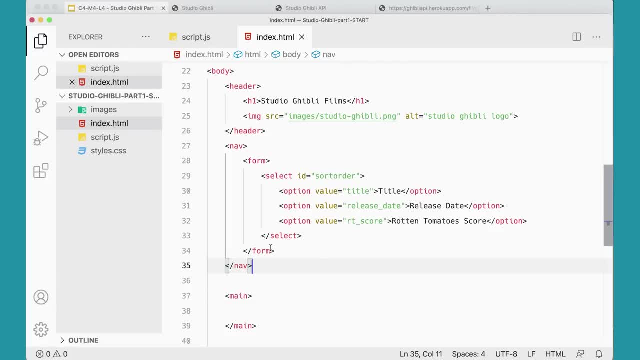 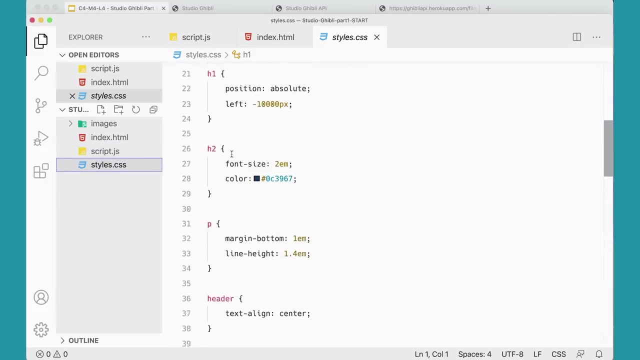 So we've added that to the file, Save that. And then we also want to add a little bit of CSS to the style sheet. Switch over to the styles here. I'm just going to scroll down the page. You can put this really anywhere, as long as it goes above the media queries here. 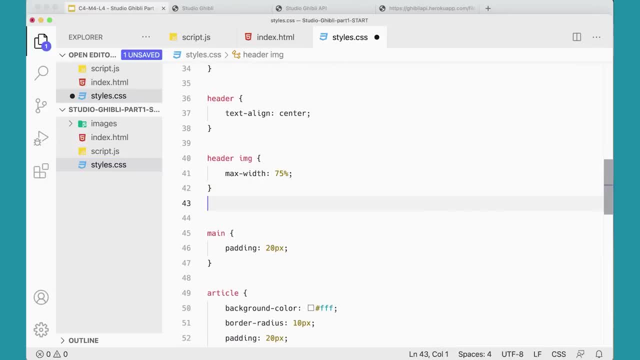 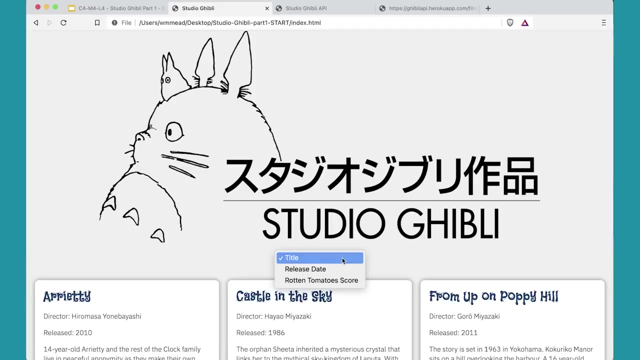 But I'm going to stick it after my header stuff, since the navigation comes after the header on the file. I'm going to just put it there And let's go over and just see if that's displaying properly. Refresh. Now I have a little list that I can actually pick from. 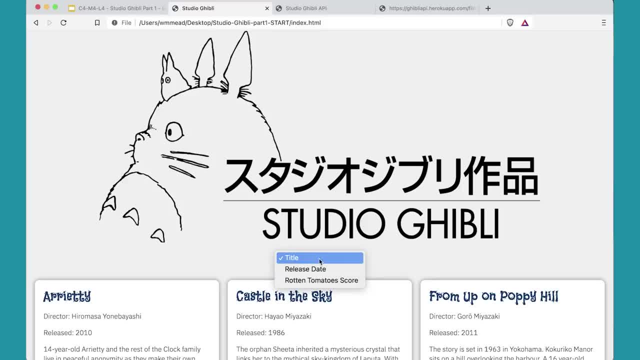 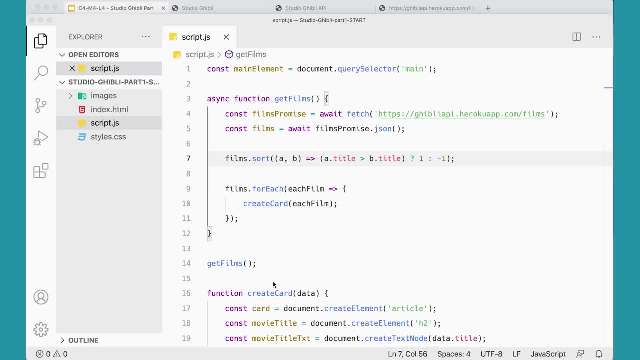 Here for title, release date and Rotten Tomatoes score. So that's pretty cool. Next, I'm going to add an event listener that will listen for when this form changes here. So this form doesn't have a submit button or anything fancy like that. 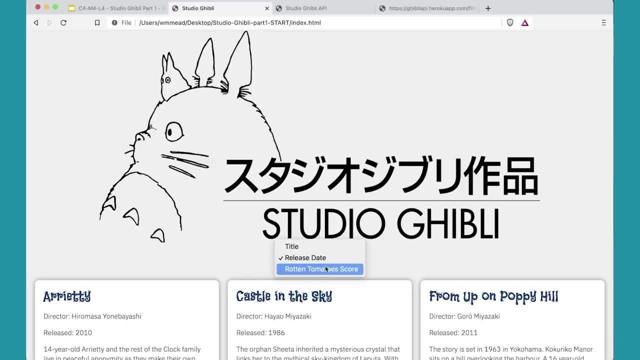 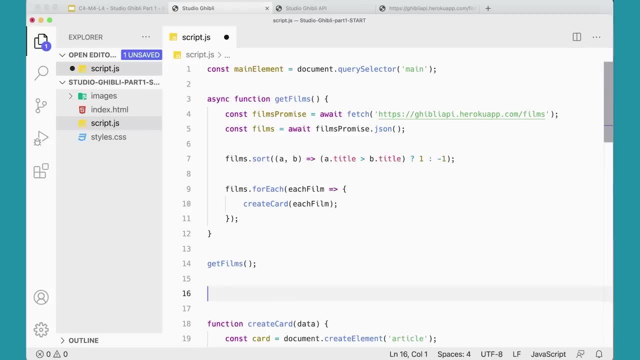 I just want to know if somebody chooses release date or Rotten Tomatoes. I want to know when this list changes. So let's see if we can write some code to affect that. So down here I'm just going to click and press return here. 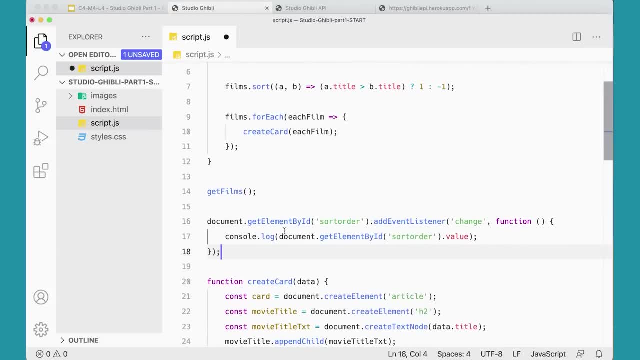 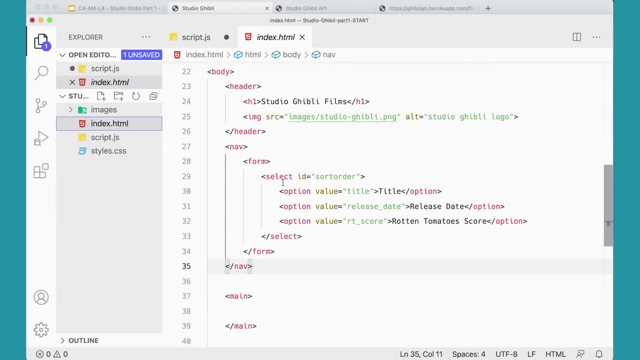 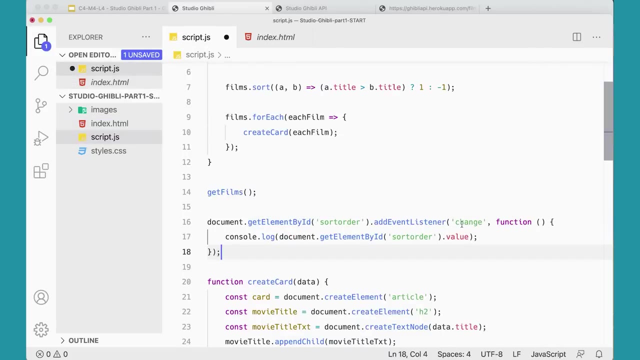 I'm going to add this Document, get element by ID sort order, Which is again this select list, ID select list. So I'm getting that ID sort order And I'm adding an event listener And I'm listening for a change. 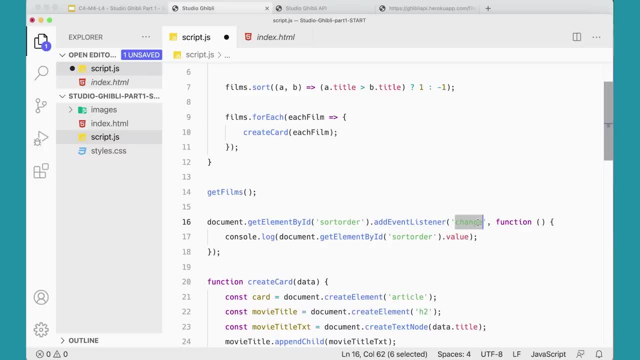 So I'm not going to change that. I'm not listening for a submit, for a submission of the form. I don't have an actual submit button or anything like that. I'm just looking to see if it changes. When it changes, I'm going to run a function. 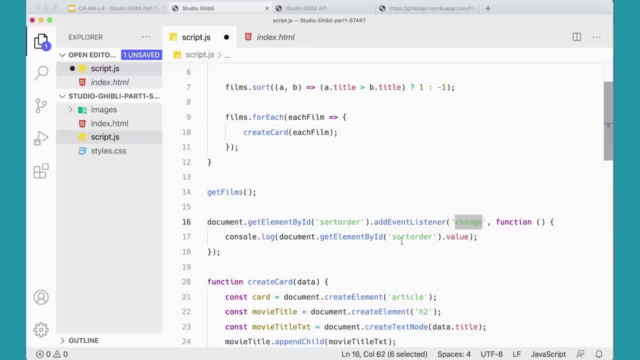 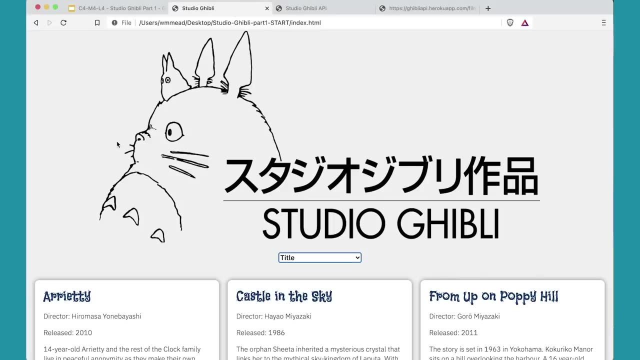 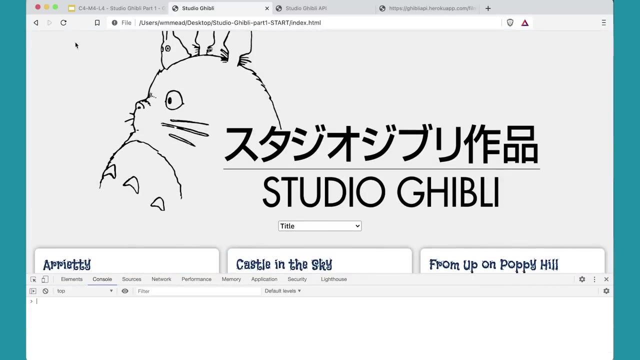 And for right now I'm just going to console log out the value of that sort order. So let's just save that and see what happens over here when I'm going to turn on my inspector And go to my console here And I'm going to just refresh the page real quick. 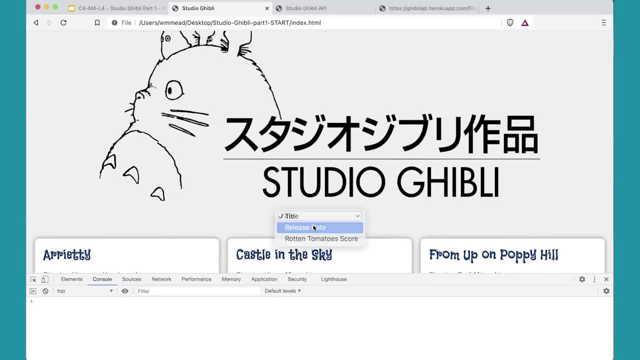 And now, if I click release date, you can see I get release date there, So I can capture when this is changed. Aha, that's a good clue. If I can capture when this is changed, I can take these values and do something with them in JavaScript. 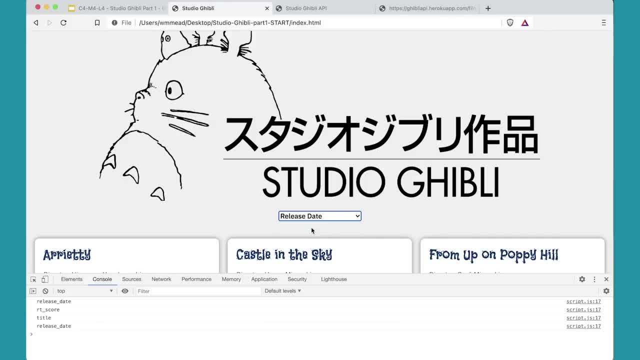 So this is giving me some input that I can do something with in JavaScript. And if you're wondering, like, what's RT underscore score other than rotten tomato, Rotten tomato score? You know where is it getting that. Just remember to go look at the HTML. 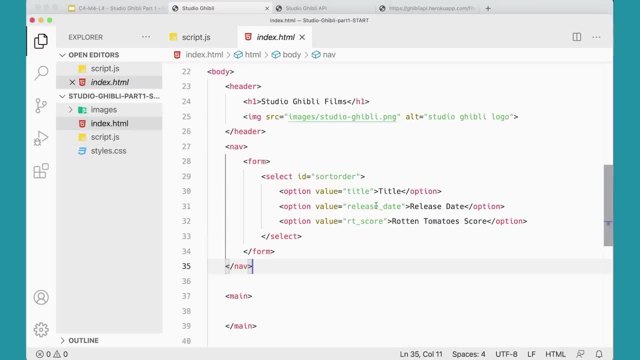 And you can see these are the actual values that are being sent: Release underscore date And RT underscore score- And it's important to note that I've set it up this way because this matches the actual data that we're getting from our API. 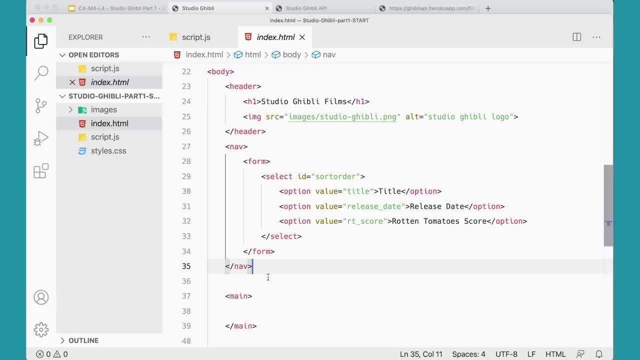 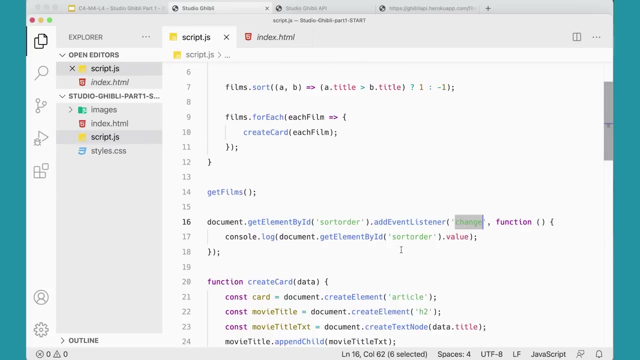 So that's helpful as well, Great. So now we've got a way of capturing that stuff, And it would be kind of nice now if we could have a function that would allow us to sort based on these different values that we're getting here. 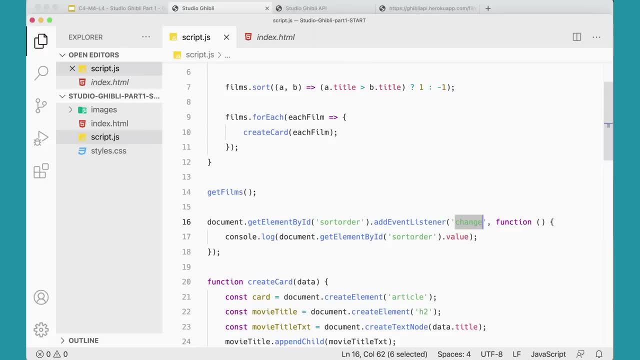 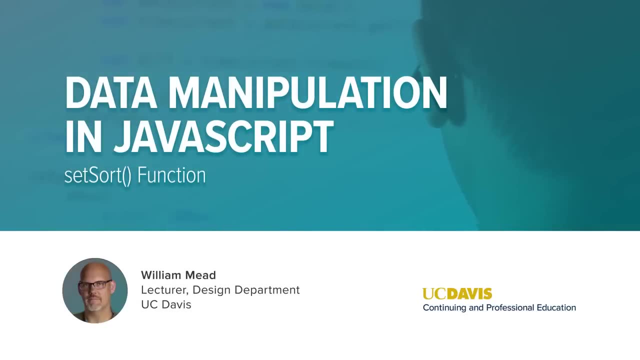 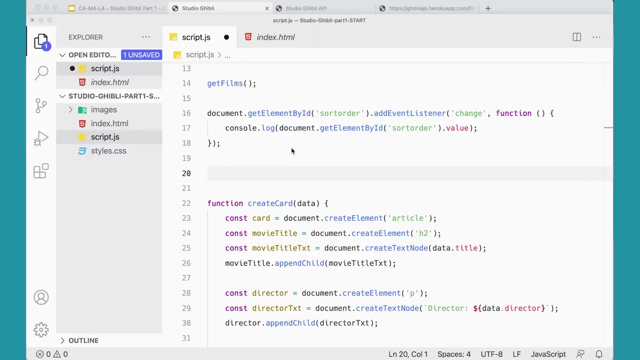 And we'll take a look at that in the next video. In the previous video we saw that we could create a list, a select list, And then, when that select list changes, we could grab the value that it's changed to. So now we need to add a function called set sort. 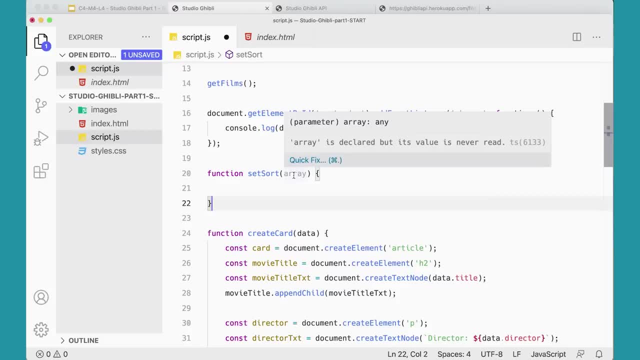 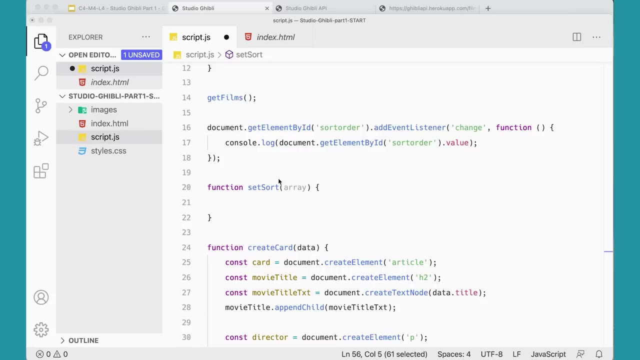 And it's going to take an array of items, And then we're going to sort them based on some different criteria, based on what gets set here. basically, That's the criteria we're looking for. The first thing we need to do is to get the value of what it is that was set there. 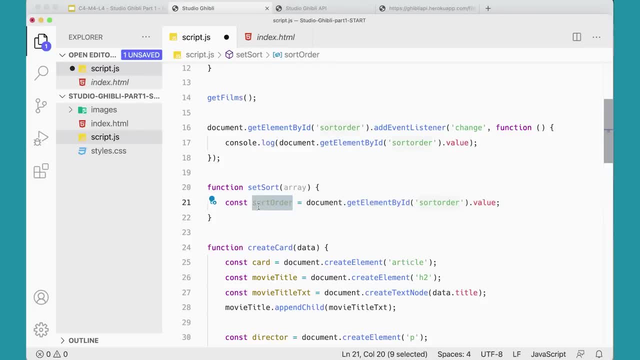 So I'm going to make a value, a variable called sort order, And it's going to just go in and get the value of whatever that select list is set up And I'm going to set that there And then I'm going to use a switch statement: switch. 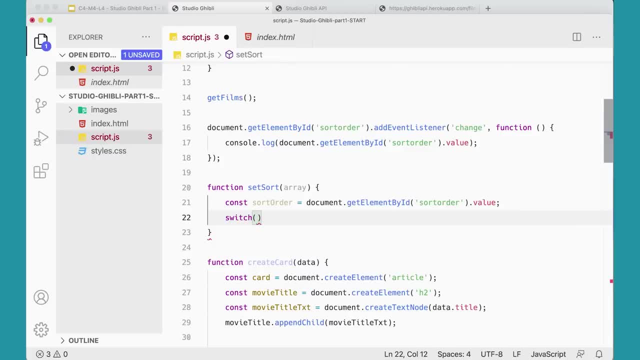 And you could use a series. You could use if-else statements or other kinds of- yeah, you could use if-else statements if you wanted to, But I like switch because it's nice and compact And I want to check the value of this sort order here in switch. 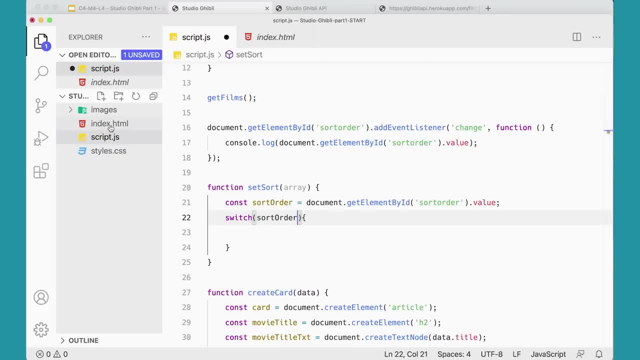 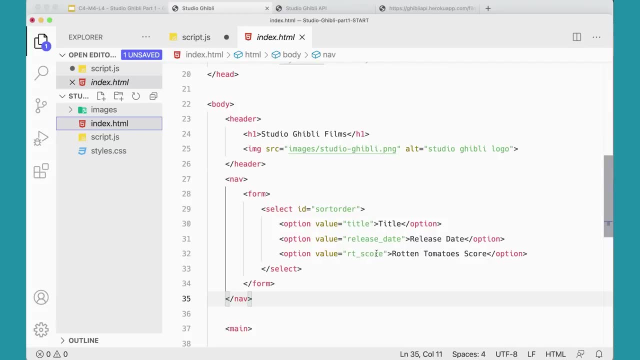 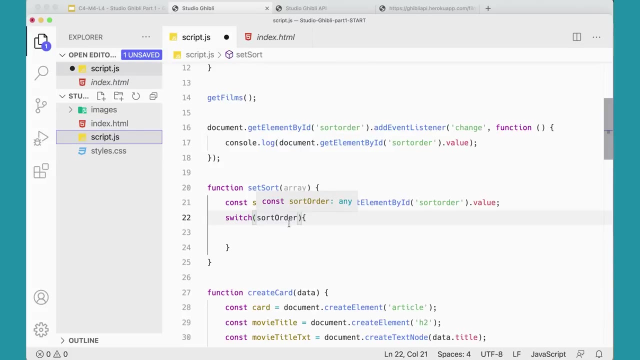 Because it's either going to be- it's going to be one of these three things- It's going to either be title release underscore date or RT underscore score, Like that. It's going to be one of those three things. So, depending on one of those three things, I want to do something with it. 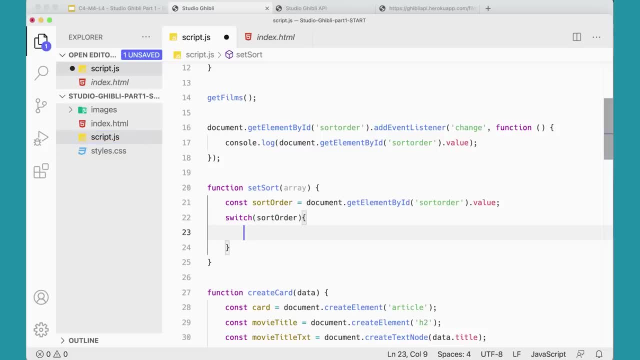 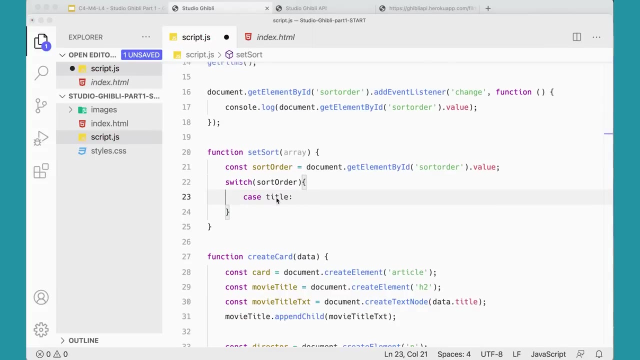 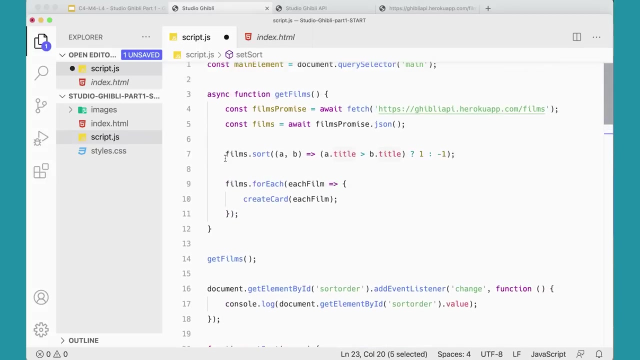 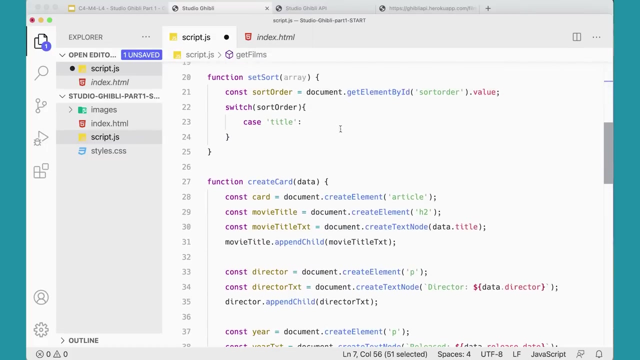 In case it's the title: case title like so, And whoops, that's got to go in quotes In case it's the title. In case it's the title, I want to essentially do this Right, But instead of films, I'm going to pass in array whatever I get passed in here. 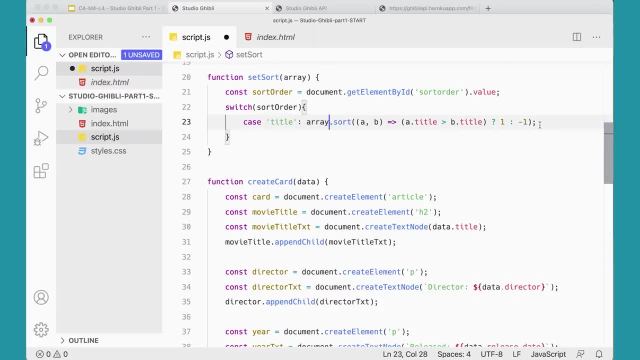 So I want array there instead, Like that, And then when I get to the end I need to remember to do break on the line. So that's for the title, In case it's the title, But then I need two more lines to handle my release date and my Rotten Tomatoes score. 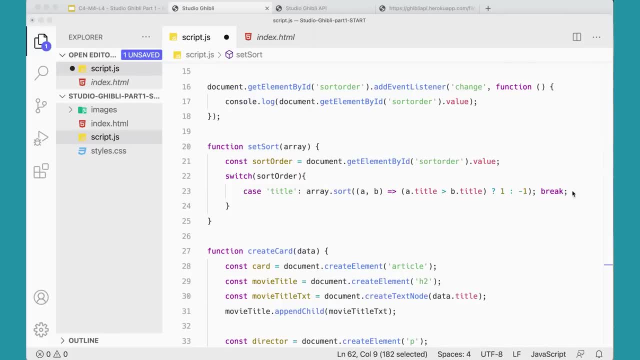 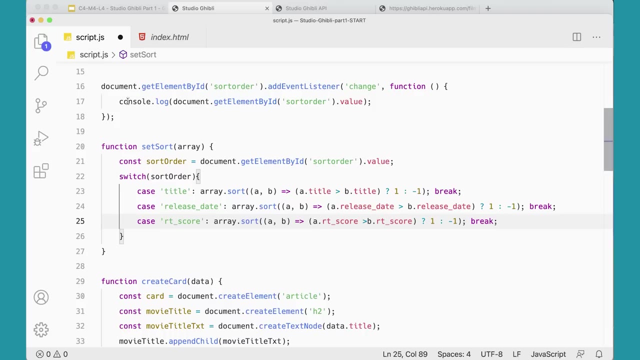 And they're going to look like this. Release date: Rotten Tomatoes score. And you can see they're very similar. It's wrapping around kind of funny. I'm going to close this thing so you can see it better. Release date. 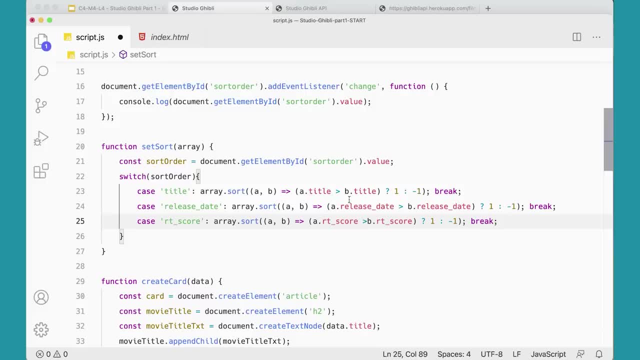 It's basically the same thing. I'm just doing array, sort, And then I replace title with release date, Release date And break there. And then down here, Rotten Tomatoes score, Rotten Tomatoes score, Like that there. 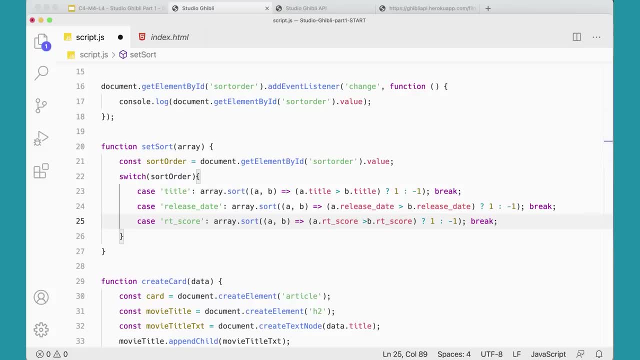 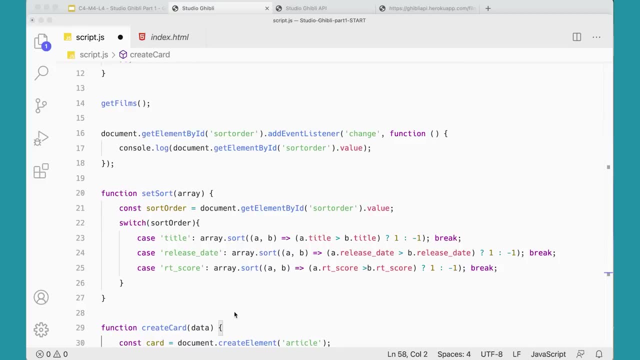 Okay, So that's all good. Now here's your challenge, Here's your micro challenge to work on, And I really recommend trying to do this without going forward. Try to do this on your own, Because this is a great sort of micro challenge: to figure out how to put these pieces together. 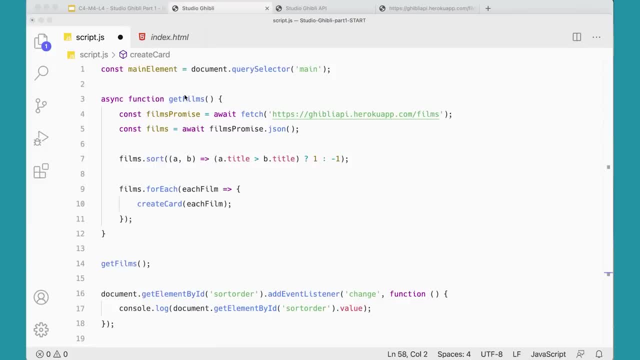 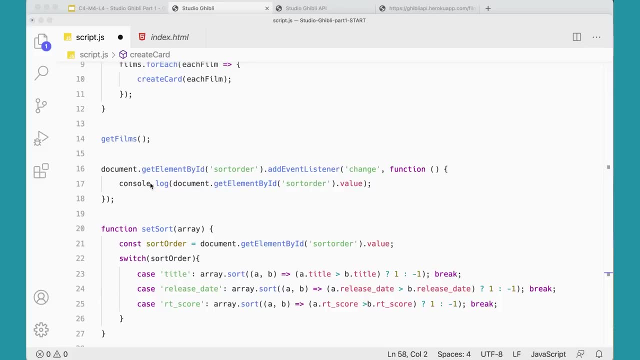 You have a function that gets the films. That's this function up here: Get films. You have a function, or you have this event listener that detects when the form is changed, And at this point We're just console logging out the fact that it's changed. 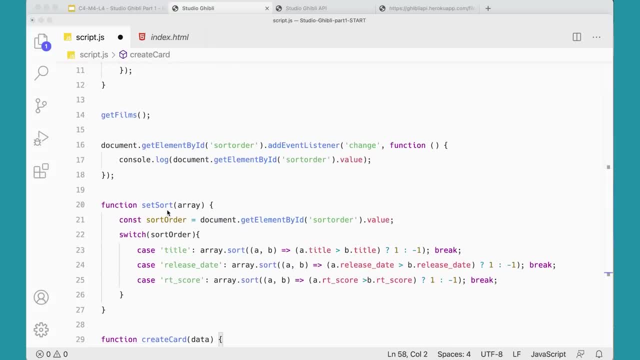 And we have a function that will actually set the sort based on an array that you put into it. What do you need to do to make these three different pieces work together- This function, This event listener And this function up here. What can we do to kind of make these three things work together? 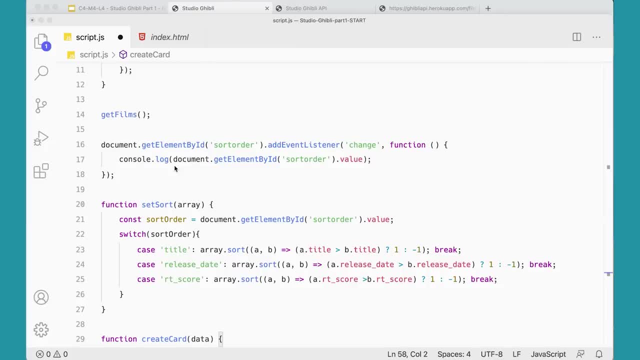 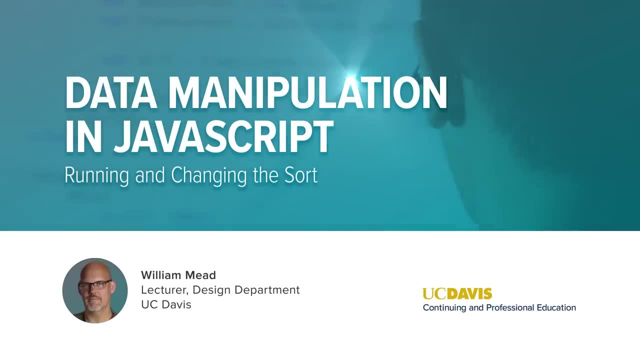 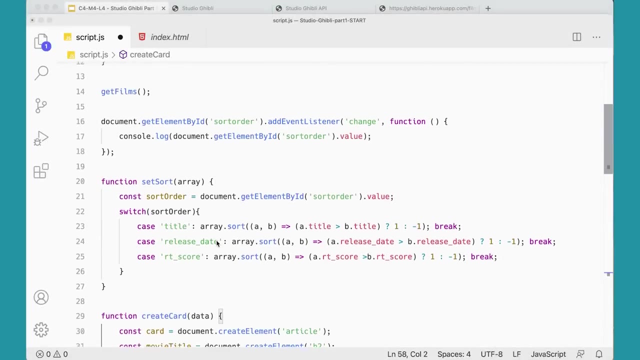 See if you can figure that out on your own, And in the next video we'll do it together. In the previous video we were able to create these separate pieces here. Now we needed to put them together. Were you able to do that? 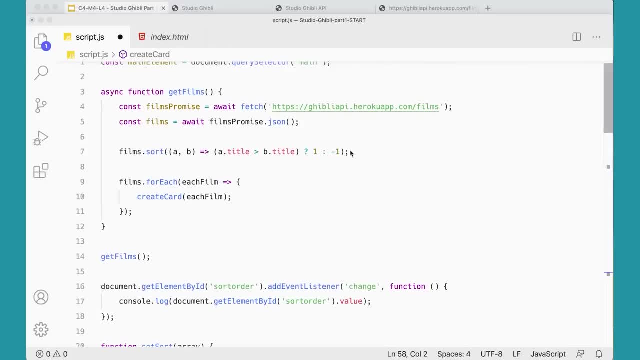 Let's see what you did. This is what I would do. I'm going to remove this from up here And instead I'm going to run my set sort Function here. I'm going to pass in the films array. Did you get that? 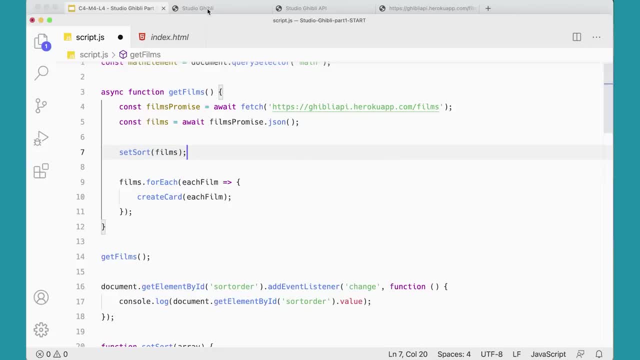 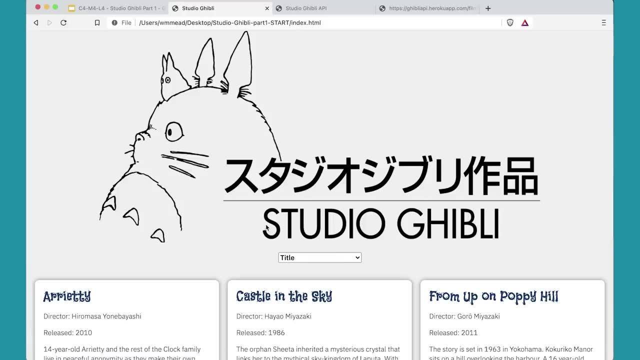 Because when the page loads this page here, when it loads by default, the title will be set. If I click refresh here, The title is set by title And you can see that it's already getting, It's already working, It's getting. 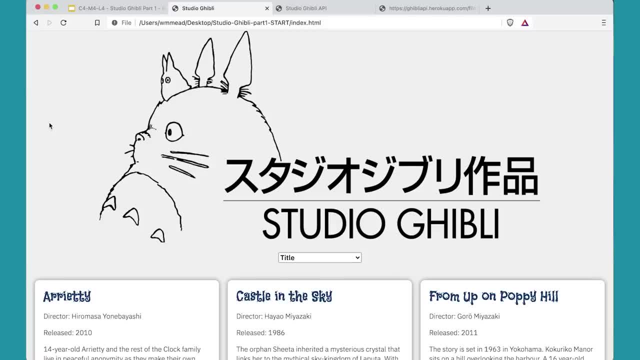 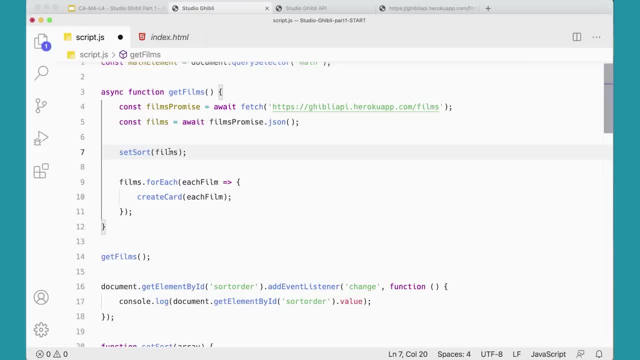 So this is the default one. It's going to automatically sort them by title if I do that, So that's great. So set sort films is going to get them. It's going to set them and get those films and set the sort. 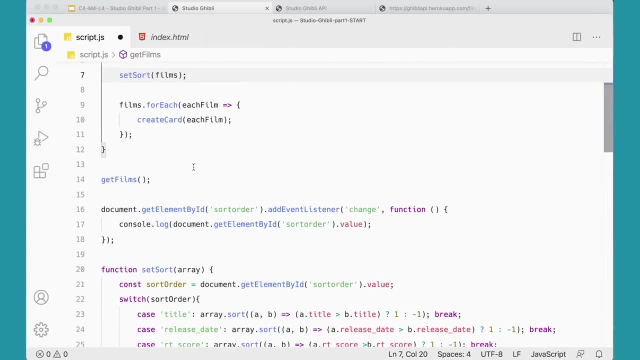 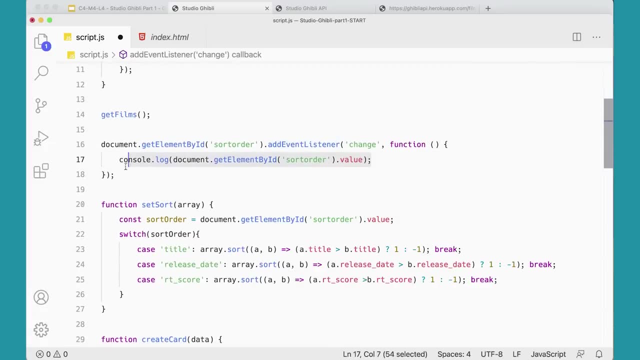 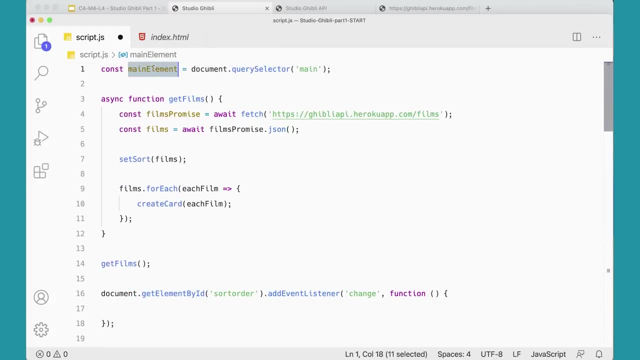 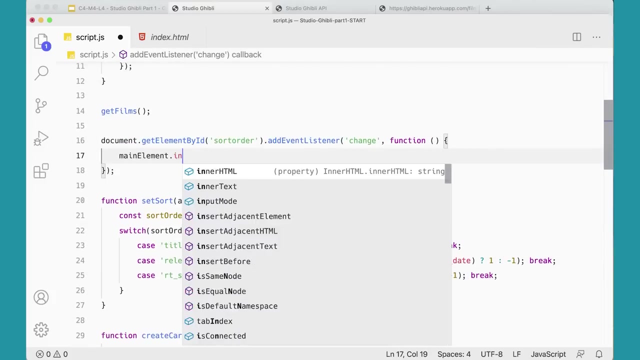 And it will automatically do it by title Plus down here. if you've changed the sort order, then this event listener fires. So what we need to do is we need to take that main element, This one here. Main element: innerHTML. 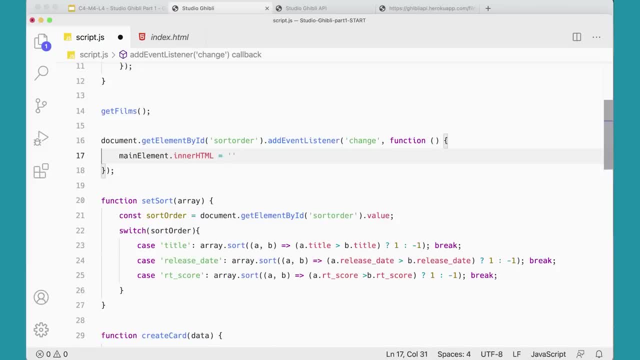 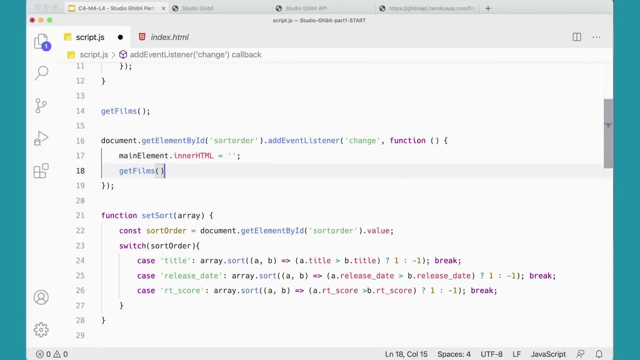 And set it to empty. Set of empty quotes there. We need to empty it out And then run, set, sort again. Sorry, I mean run, get films again. Get films here, So that will clear it out. If you don't clear it out then you'll get the films a second time. 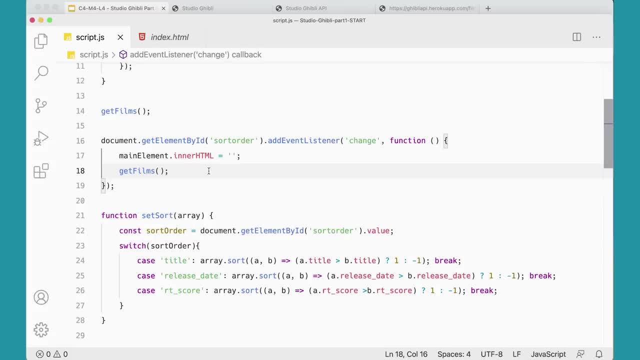 And they'll get appended down to the bottom of the page Because, remember, we're appending our cards to the main element, So they'll just get appended again And you'll get the second list of all of the films after the first list of all of the films, if you don't clear out the HTML there. 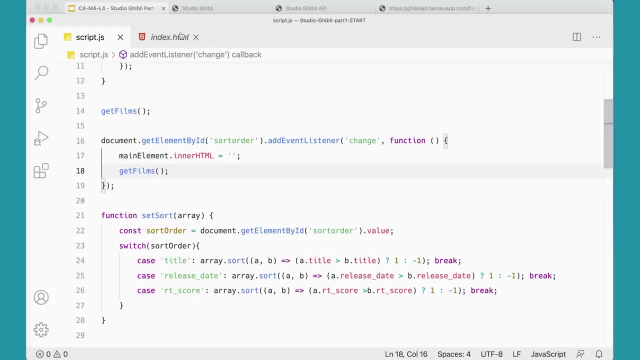 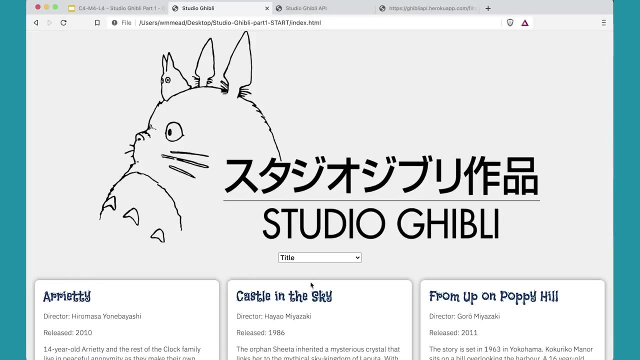 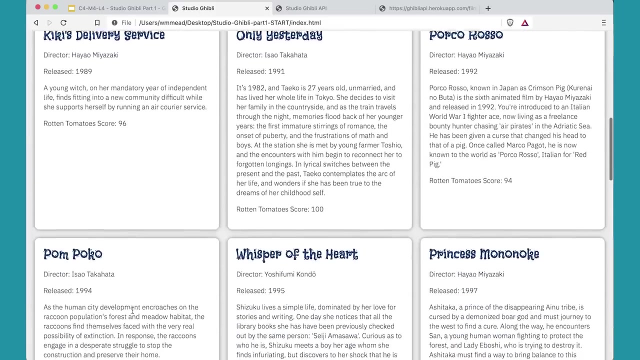 So let's save this, Make sure that's all nice and saved And test it out. Come over here, Refresh my page. Refresh my page. They're coming in by title. If I choose release date, I'm getting them by release date starting in 1986.. 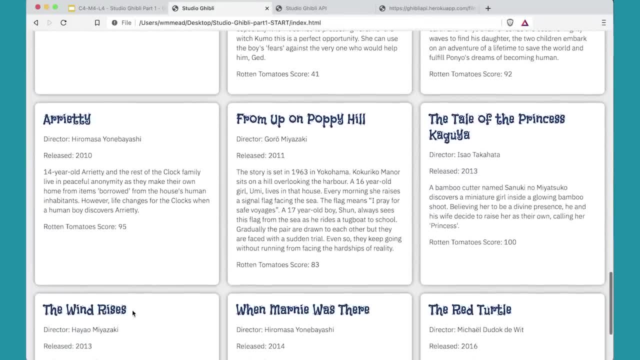 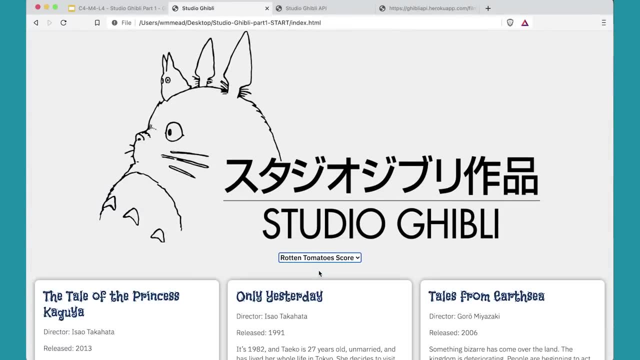 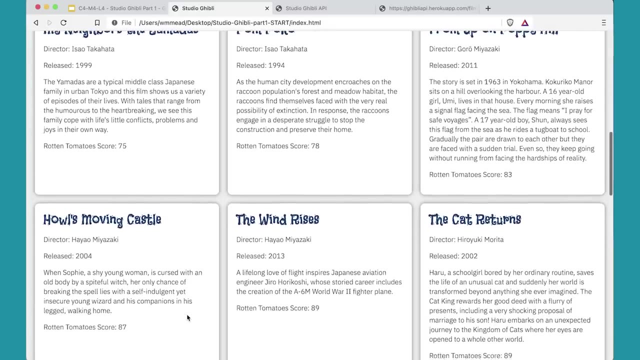 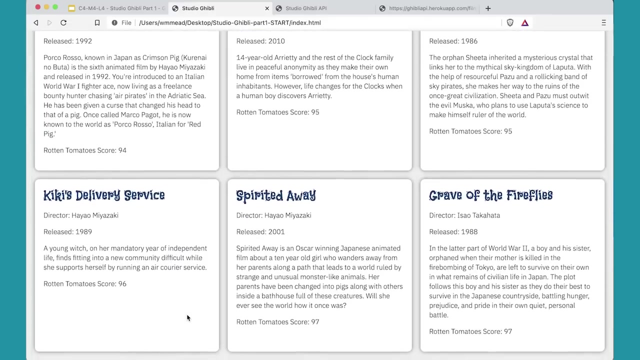 And going up to 2016.. If I choose rotten tomato score, I'm getting the highest score films first And then going down the list to the lowest score films at the bottom. I have these coming in in reverse order here. Actually, no. 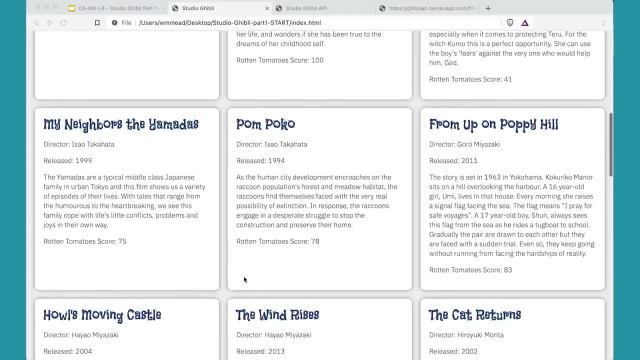 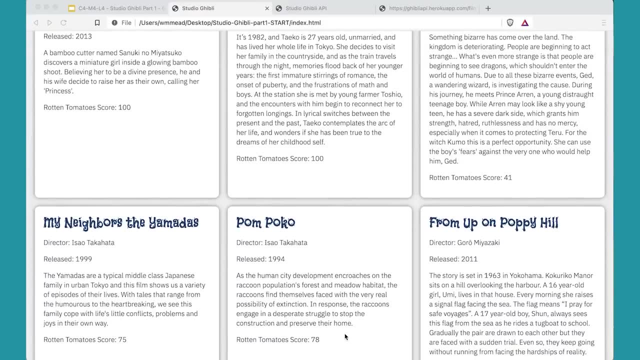 Notice, the order is a little bit screwed up. We have up at the top we have 100, 100. And then we have 41 and 75 and 78 and 83. So it's going in kind of a weird order. 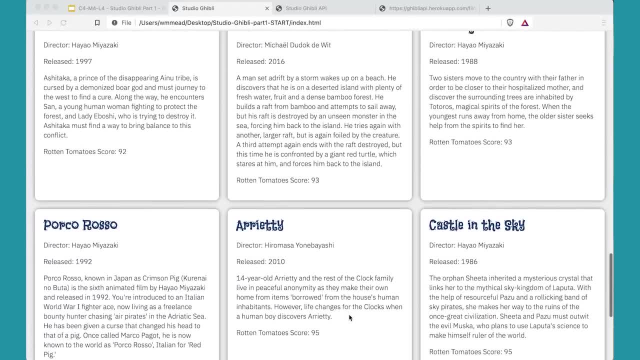 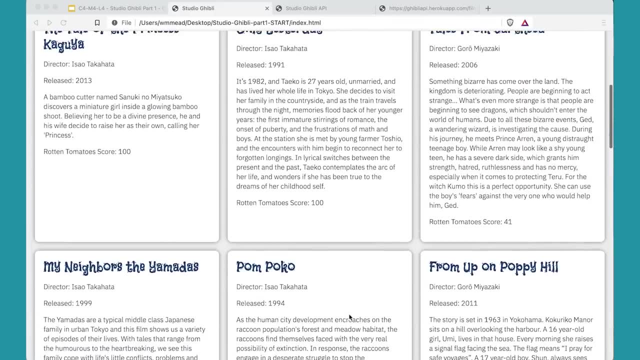 So we need to fix that. What it's doing is it's sorting these numbers alphabetically, So 100 comes first, because it starts with 1. And then it's going to 41 and going up from there, And that doesn't make any sense. 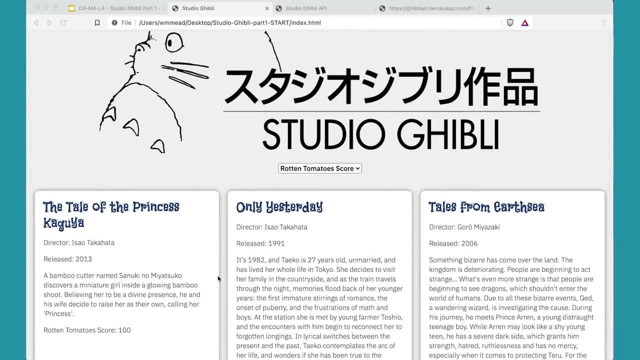 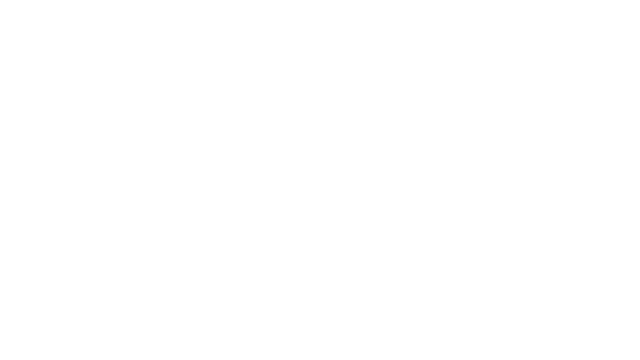 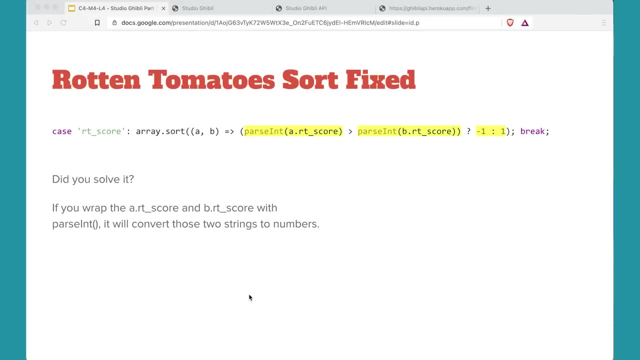 And not only that, but it would make more sense to put the highest rated movies at the top and go to the lowest rated movies. So let's see if we can fix that. Fixing this is not too difficult. What I want to do is use our old friend parseInt, so that I can take those numbers and have them get parsed as integers rather than have them automatically be treated like text. 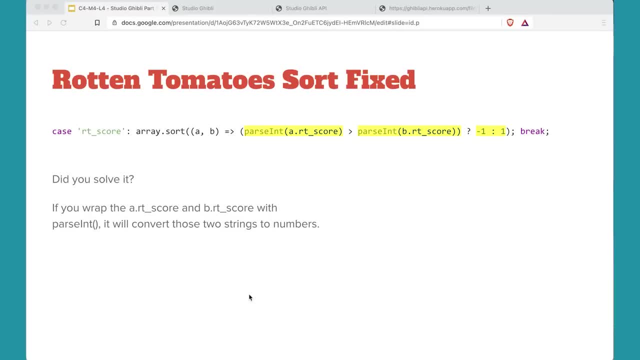 So I'm going to wrap my ART score and BRT score inside of parseInt And then over. at the end of this I'm going to swap the order, So I'm going to put minus 1 first and 1 last So that they go in reverse order. 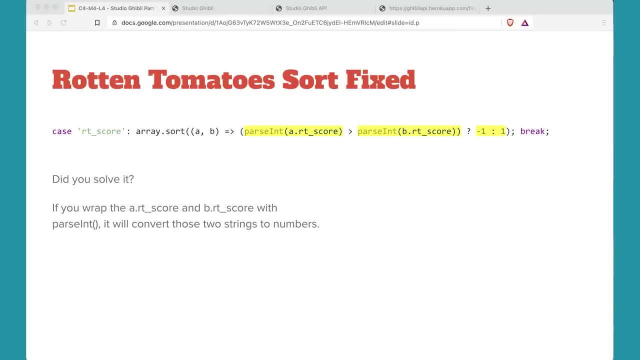 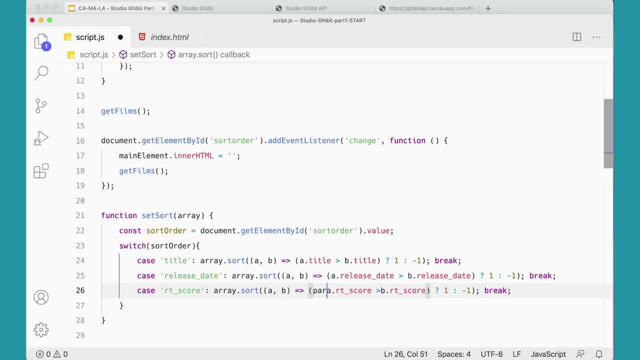 So let's go ahead and put this into our code over here. So it's kind of helpful. So down here I'm going to just put parseInt here around this one And parseInt here around this one. Don't forget we've got two parentheses here, because that one's closing this one. 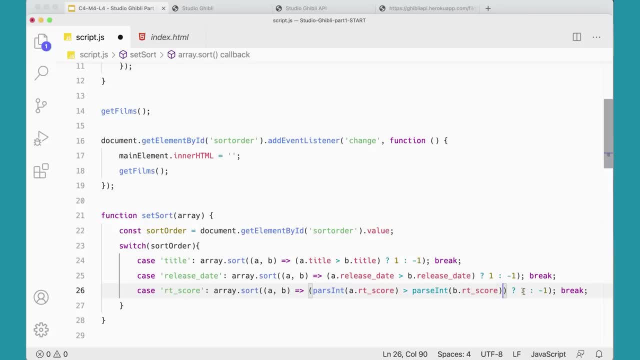 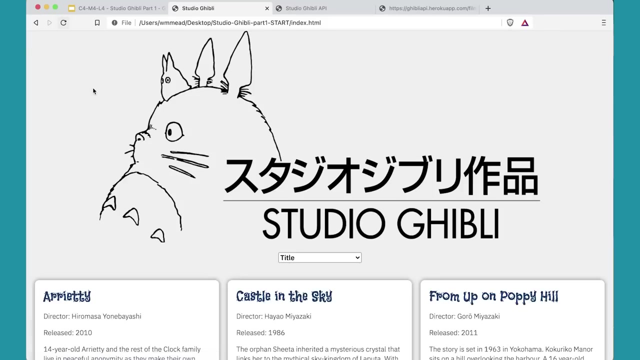 So parseInt, parseInt And then over here I'm just going to swap these. I'm going to put minus 1 first and 1 last. Save that. Let's give that a try and see if that works. Refresh the page. 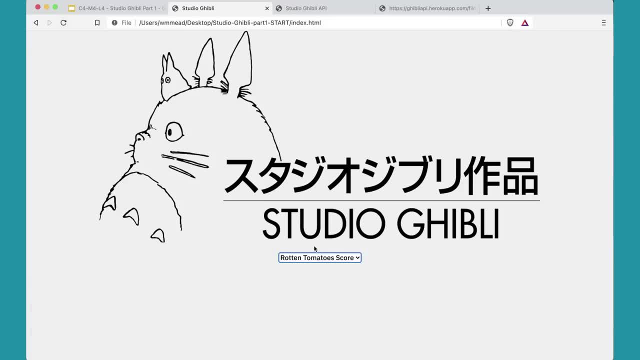 It's coming in by title. If I choose rotten tomato score, I must have made a mistake. Inspect, Always use your inspector. You can see I have an error here. Console Uncut promise. parseInt is not defined. Look at that. 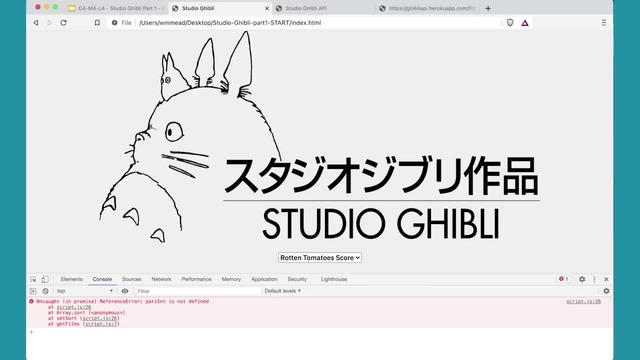 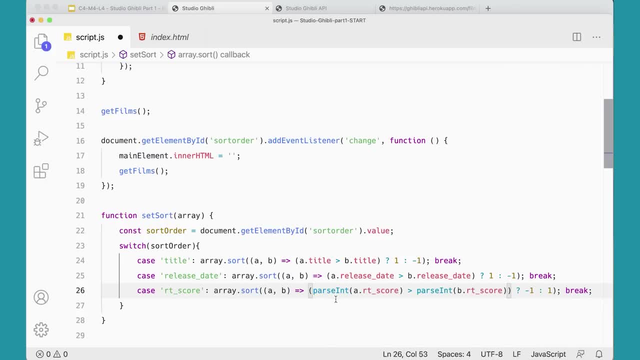 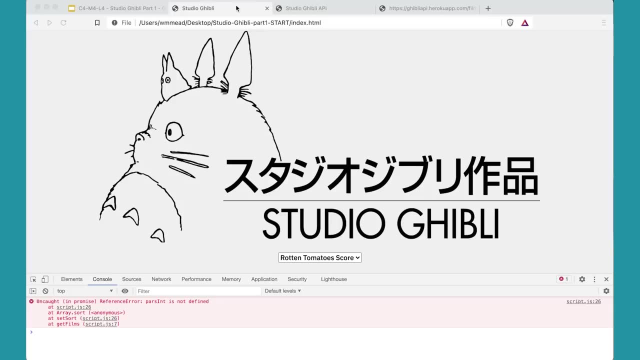 You can see right there, I misspelled parseInt. It's really easy to do this kind of thing. ParseInt, That's not a function. Parse without an e is not a function. ParseInt Like that. Let's try it again. 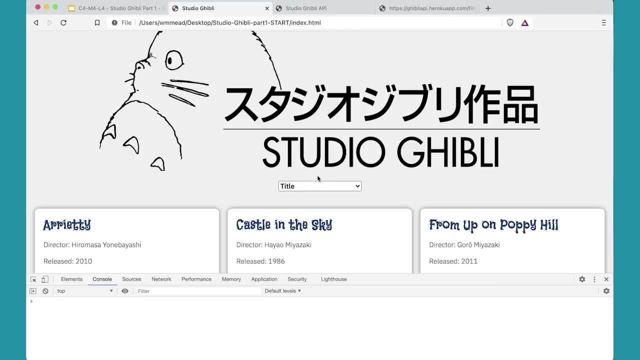 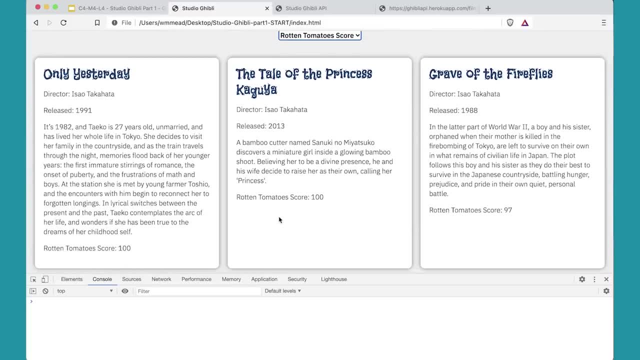 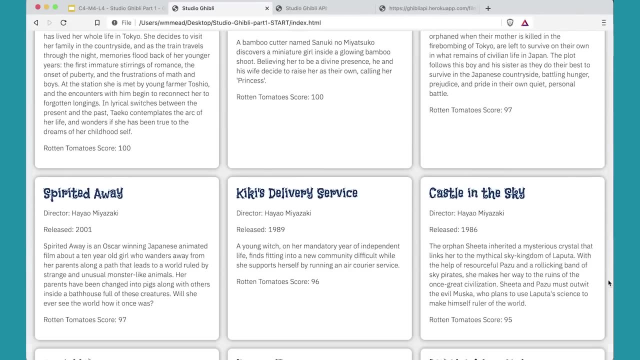 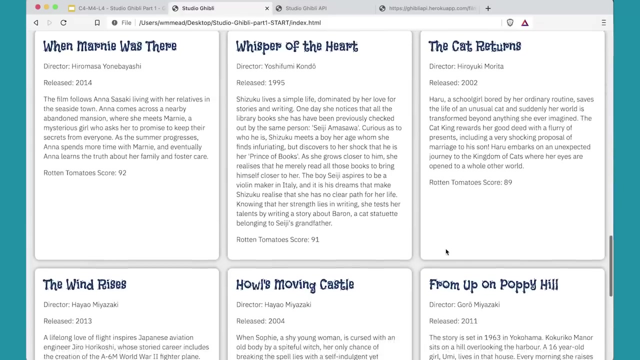 Refresh By title. they're coming in fine. If I choose rotten tomato score Now, I've got 100 first, 100 second, 97, third. Close this inspector: 97, 96, 95. All the way down to the end here. 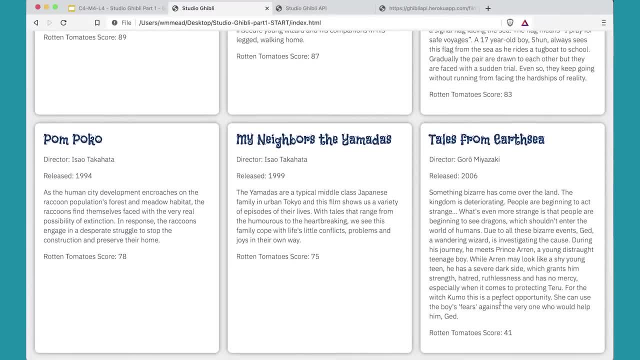 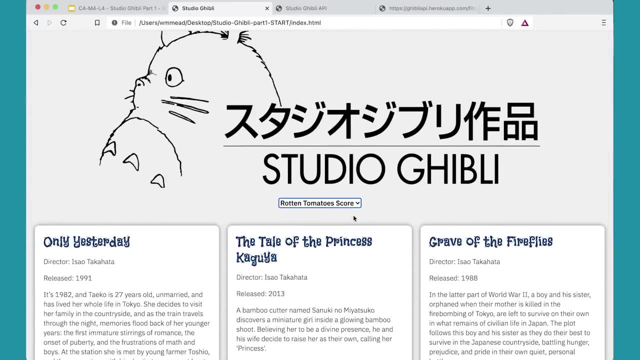 41 will be last. So that's working great. All right cool. So we've got all of our films And we've got our little feature for sorting them, which is pretty nifty, And that's looking really great. All right cool. 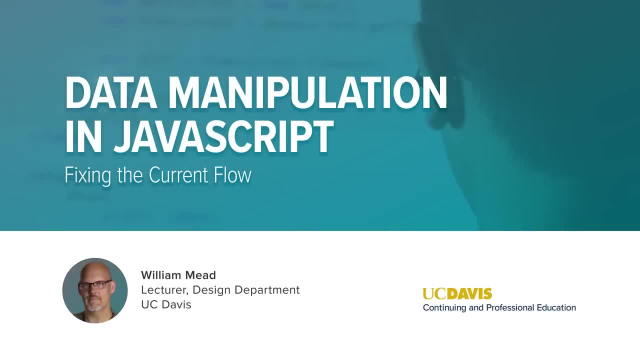 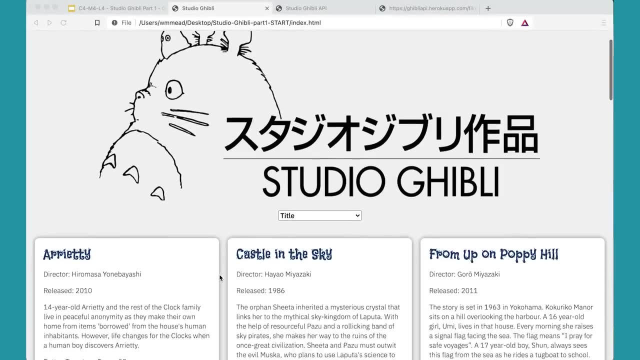 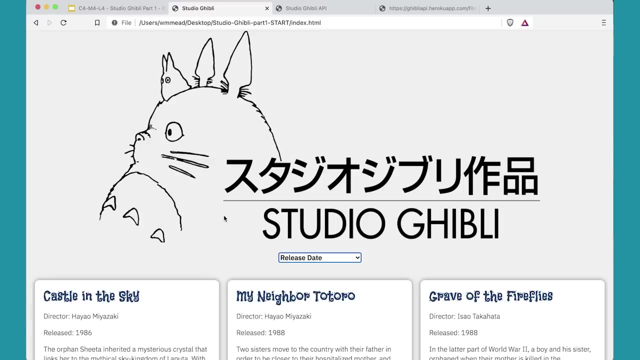 Now, there's one thing that I don't really like about our current flow for the way our page is working for this page, And that is that when I choose a different sort, like release date, I'm essentially going back to the API and reloading all of the data again. 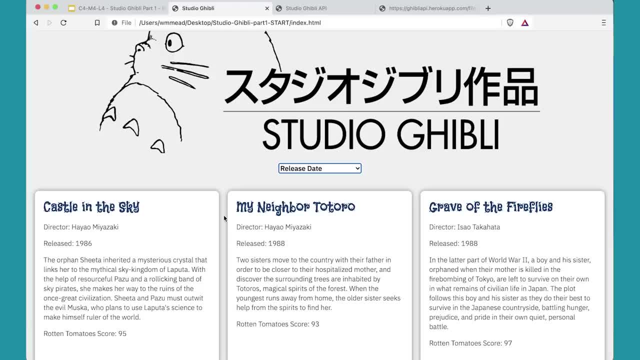 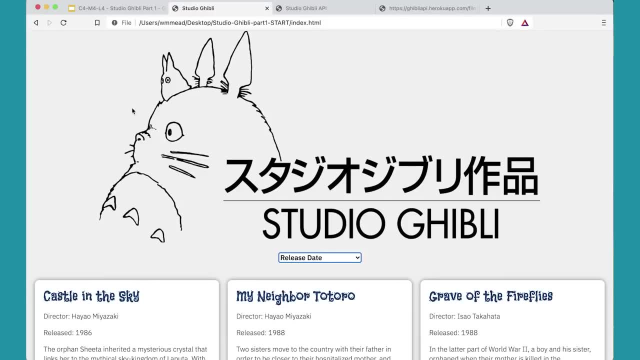 I've already gotten it once, Why should I have to go back and get it again? That seems kind of inefficient. So let's take a look at this And sort of think about what we could do to make this a little bit more efficient and a little bit better. 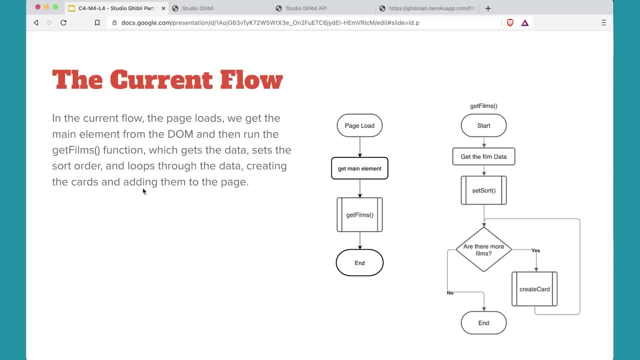 For the current flow. when the page loads, we get the main element from the DOM and then run the get films function which gets the data, sets the sort order and loops through the data, creating the cards and adding them to the page. 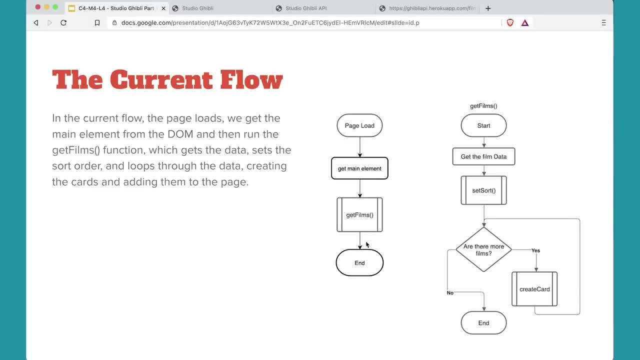 We can see it over here: Page load: get the main element, get films, And then the get films function gets that film data, sorts it. Are there more films? If yes, we create a card And we do that until all the cards are created. 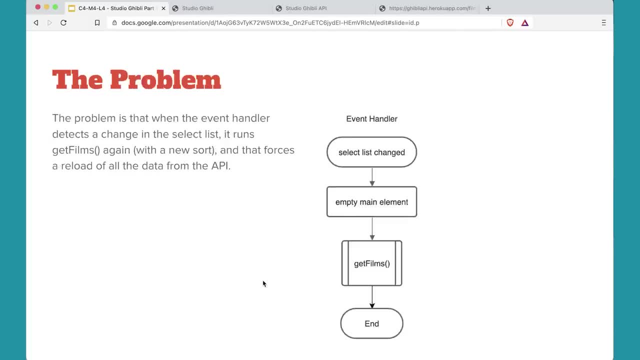 And then we end. That's the current flow. Here's the problem. The problem is that when the event handler detects a change in the select list, it runs get films again with the new sort And that forces a reload of the data from the API. 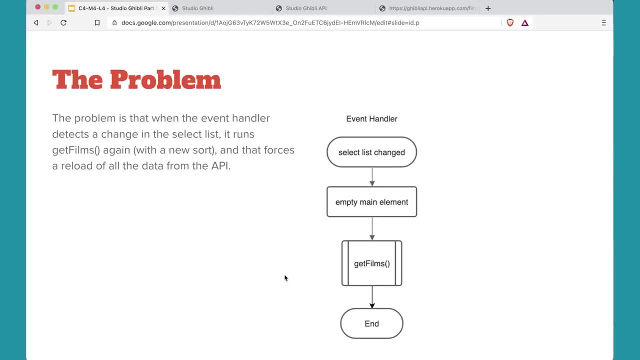 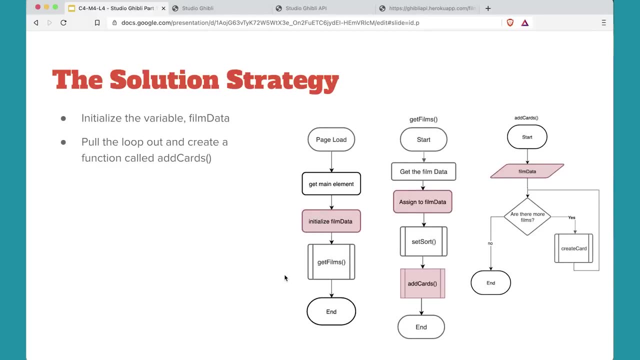 That's kind of inefficient and messy. Here's my solution strategy. When the page loads, I'm going to initialize a variable called film data. It starts as empty. That variable is going to be empty to begin with. Then, when get films is called and the data is retrieved from the API, it's assigned to that get film data variable. 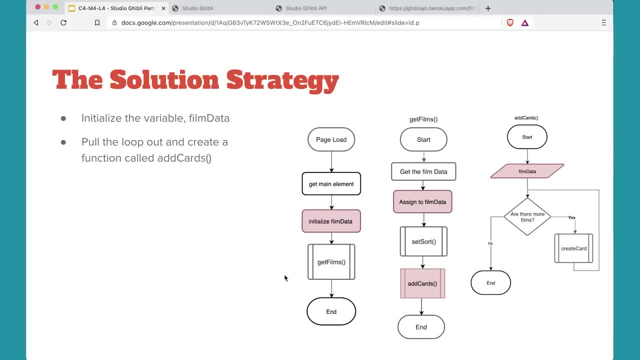 That film data variable Which started out as empty. Then, instead of looping through the data directly in the get films function, the loop is pulled out into a function called add cards Which takes the data from the film data variable. So now we're going to add one more function over here that's going to sort of pull out that process of just adding the cards. 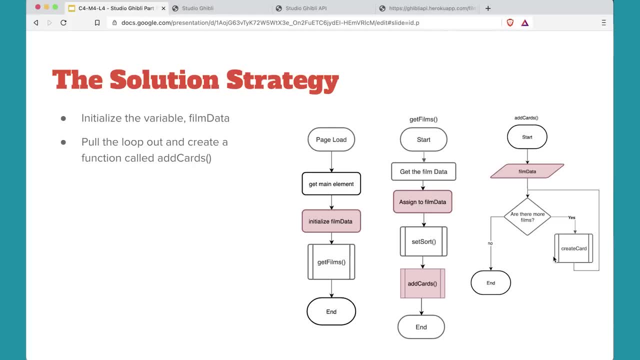 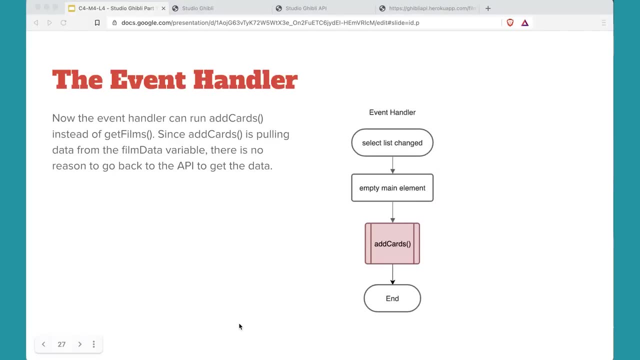 So instead of doing it all at once in the get films function, we're going to have a separate function Just for that. Then in the event handler that we use to check if the sort order is changed, Well, you will run add cards instead of running the get films function again. 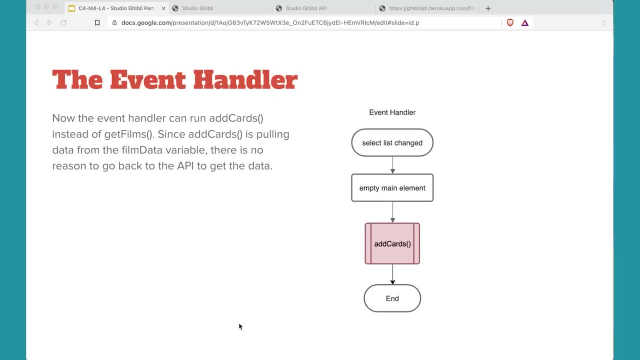 And since add cards is pulling the data from the film data variable, there's no reason to go back to the API and get the data again. It's important to note that if the data in the API were being updated frequently, you wouldn't be getting any of these updates. 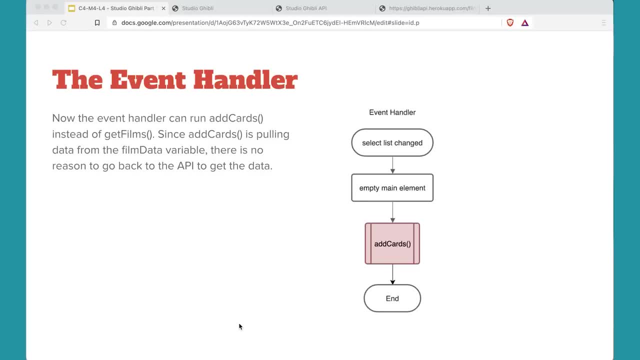 Because we're basically loading the data once and then using it, And in this case that's pretty efficient. There may be situations where you want to get the data, kind of every time you make a change or do something, you want to get the data again. 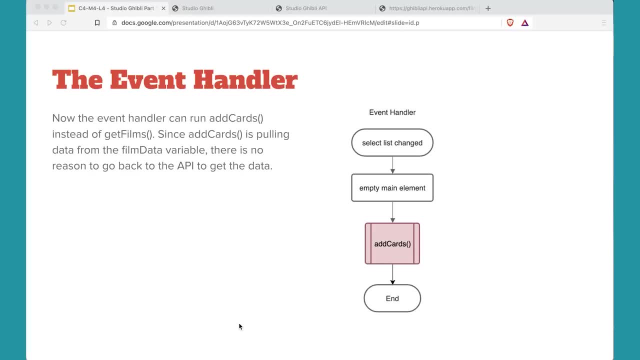 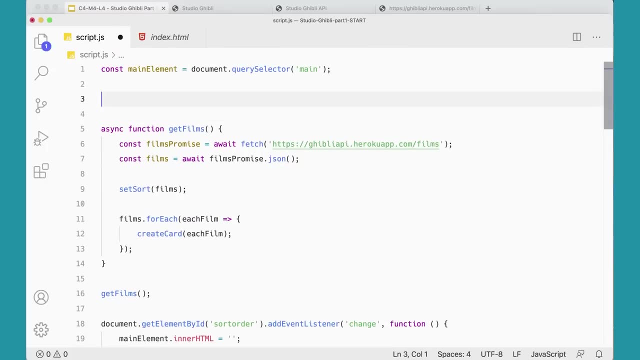 But in this case I think it's kind of nice and useful to do it this way. Back in our code. let's go ahead and add let film data. It's just a variable that is basically undefined. We're defining it, but it doesn't have any value in here yet. 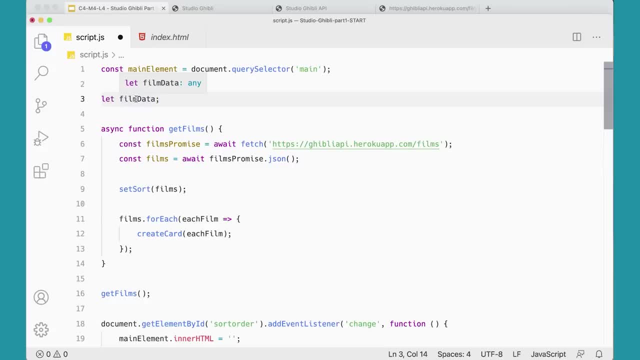 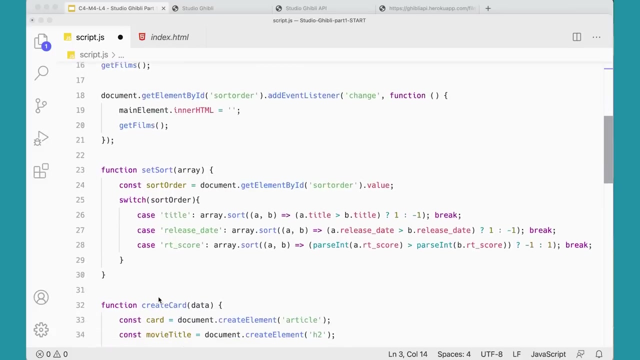 And we're using let because we're going to be adding data in there, So we can't use const, because then we wouldn't be able to change that variable. Then we need an add cards function. I'm going to stick it down after the sort. 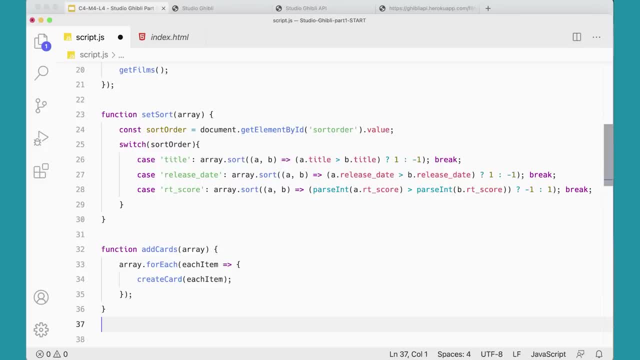 I'm going to put it here. It doesn't really matter where it goes, But I'm pasting this in here. You're going to have to type it, But I've got a function: add cards. It takes an array as a parameter and then a loop through the array and each item in the array. 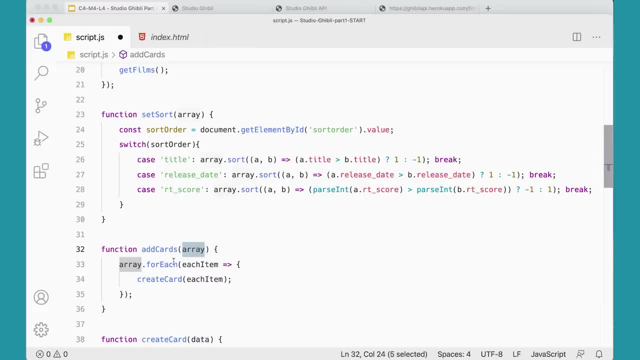 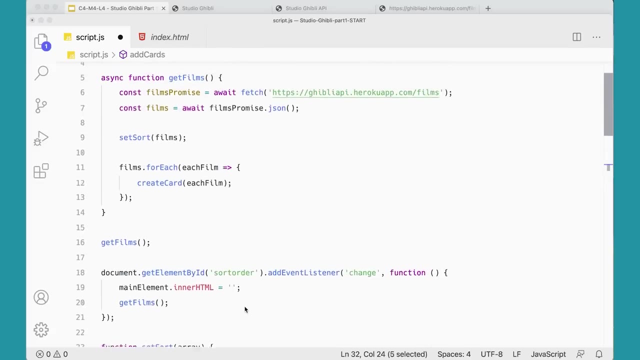 I'm going to run the create card function which is down here, So it's just a simple little helper function here That will allow us to create these create these cards by looping through an array. Now that we have that, we can go up to our get films function here. 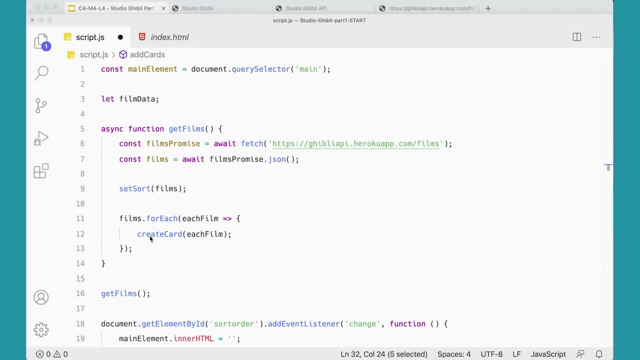 And here we're doing that same array. We're creating the cards directly here, inside of here, But now instead we're going to set our sort And then add our cards. Add cards, Films. So the first time we add cards when this function first runs. 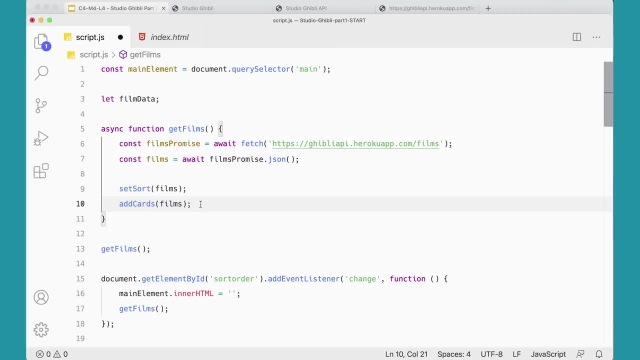 we're going to just get it straight from the data that we get from the server. But then we can say: film data equals films as well. And then, once we do that, we'll have a process for creating our logs So we can say, hey, we don't need to write all of these. 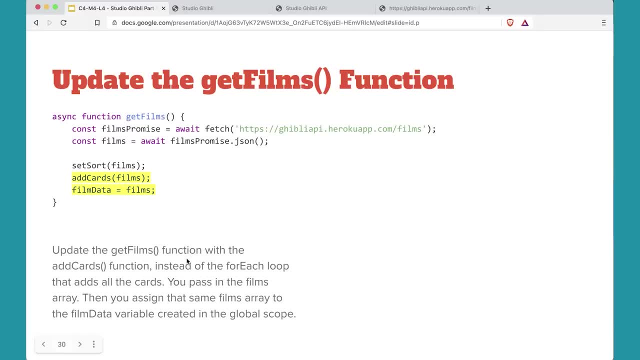 We're going to put them here And then we can say items, And then let's see if we don't have any items in our logs. We've got all of our logs there, So we can see how we're going to create our reports. 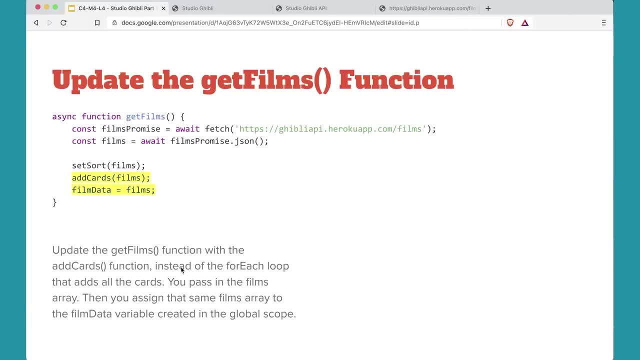 Okay, So again, I'm going to go ahead and create our logs And then, once we've created our logs, then we're going to go ahead and create our reports And then, once we've created our reports, we're going to switch to our post. 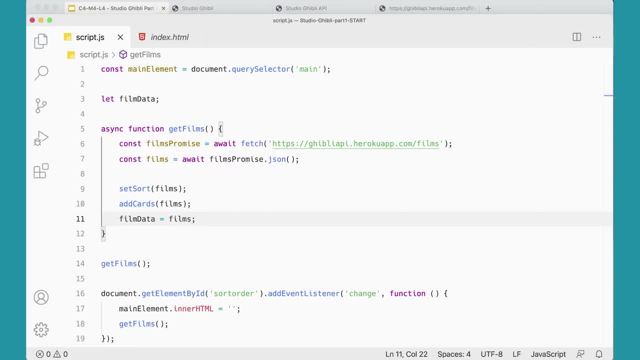 But for the moment I'm just going to click on the submit button and then I'm going to click on submit And then, once I click on submit, I'm going to go into my reports. By doing this, we've taken our films here and we've assigned it to our film data variable. 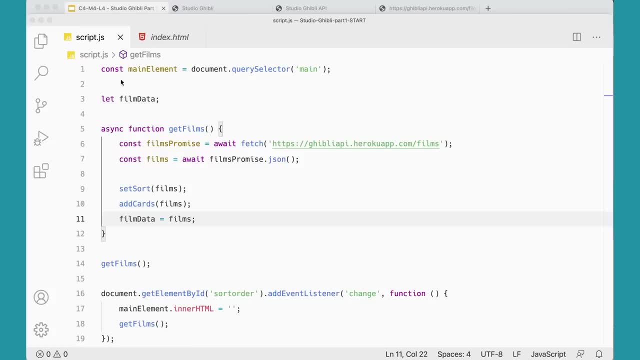 here, which is now in the global scope. We should add our IIFE function here and put everything in there, so we don't have anything in global scope. We can do that at the end to kind of clean things up, But for now we're just taking this data that we've gotten from the server and we're sticking. 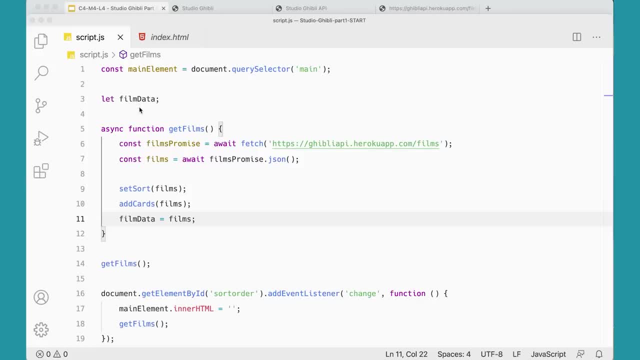 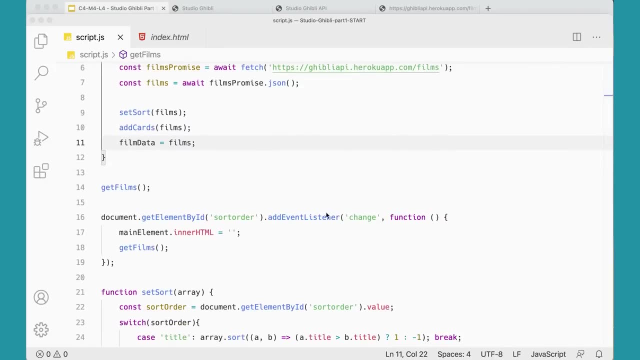 it into this variable. So now we have access to it everywhere in our script, which is super useful, And then the next thing to do is, down here in our event handler for when that changes, Instead of running, get films and going and getting the films all over again. we can now. 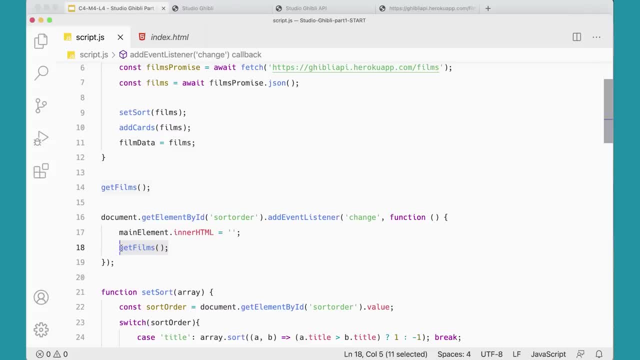 work with our film data So we can sort it, Set sort film data and we can add cards with the film data. So we're using the add cards function here to actually add the cards, after emptying out the cards that were there before and changing the sort. 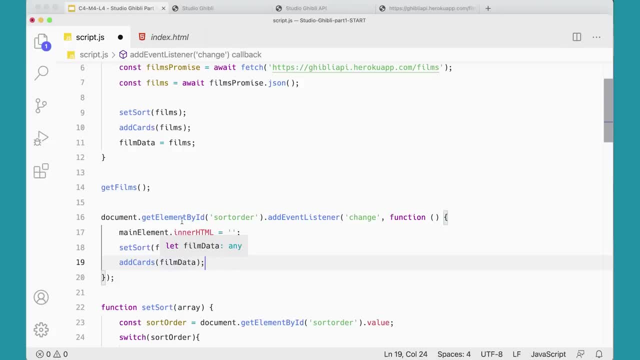 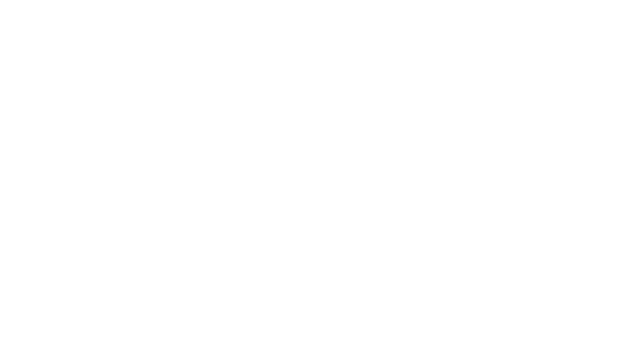 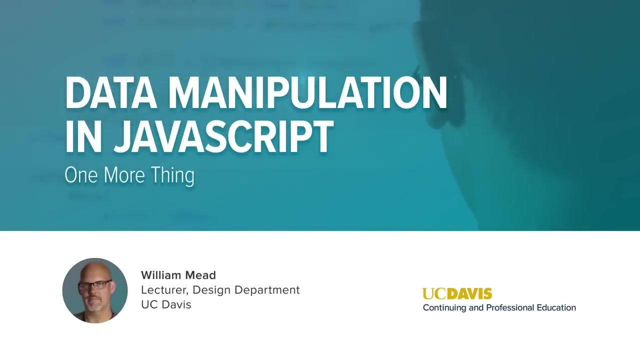 So that'll set the sort And then add the cards, But it's doing it from film data rather than going back to the API out on the internet and getting it again from there. We've gotten this pretty much set and ready to go. 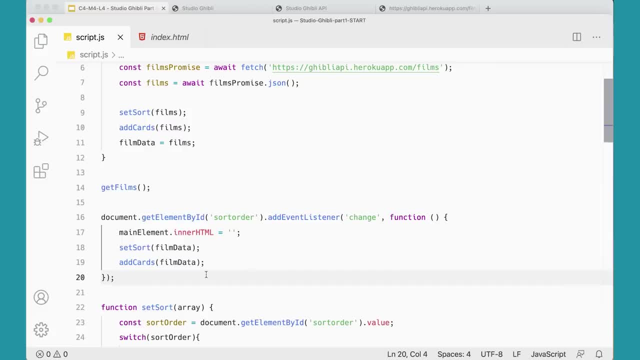 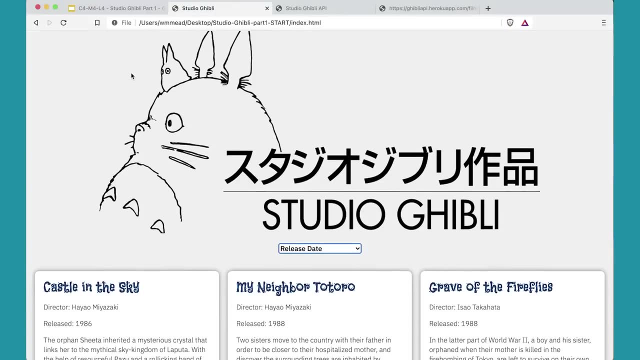 There's one more thing I want to fix, but this should be working basically here so that we can actually go and test it. If I come over here to my page here and refresh the page, it pulls in the films and you can see. it takes a second for it to load the first time. 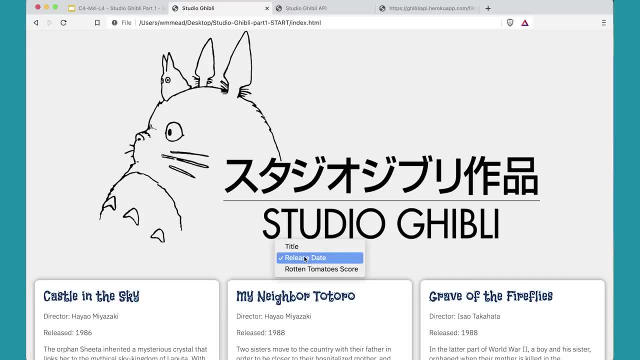 But now when I choose release date, it should go split quickly, really quickly, because now it's doing this based on the data that's already been loaded. We don't have to go and get it again, So it's running much quicker now. 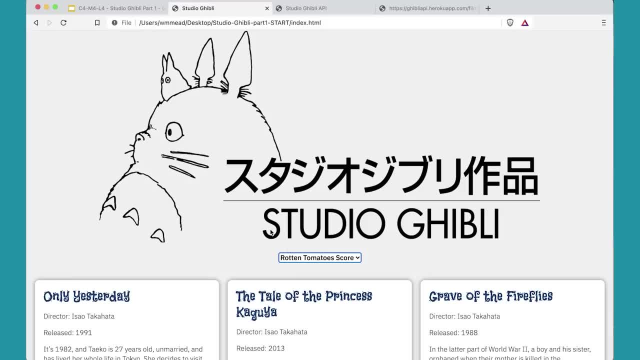 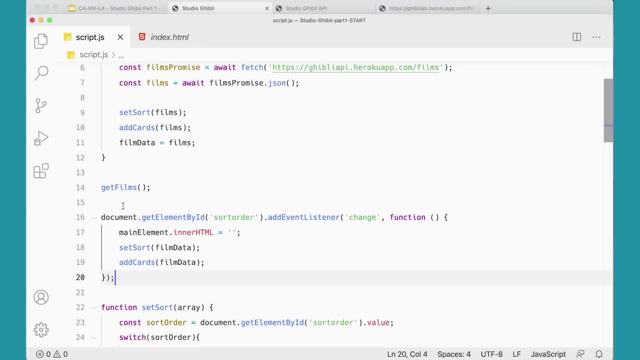 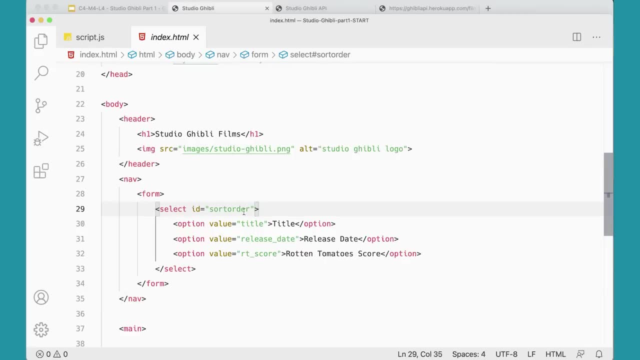 And that's great. So that's working really well. There's one last thing that I would like to fix. You come back to the code. This is just kind of a very minor thing, But I'm going to come back here. I'm going to set this select list initially to disabled- disabled so that when this page 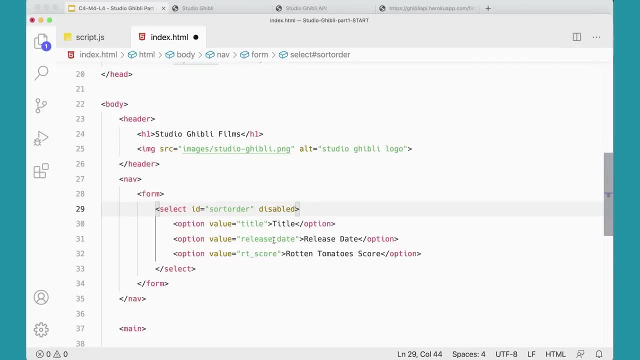 loads. this select list is disabled, And disabled- here is also short for disabled. equals quote: disabled In HTML5,. I think we've discussed this in a previous lesson. when you have an attribute that's the same as the value, you can just put in the name disabled. 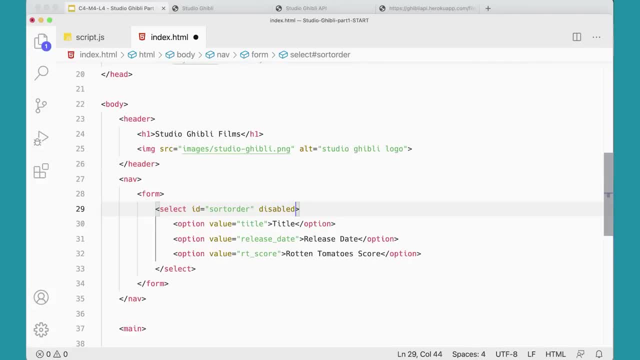 Now why would I want to do this? Why would I want to disable this? It's possible, although extremely unlikely, It's possible. It's possible. It's possible You could have a user that goes to load the page and then tries to sort the list before. 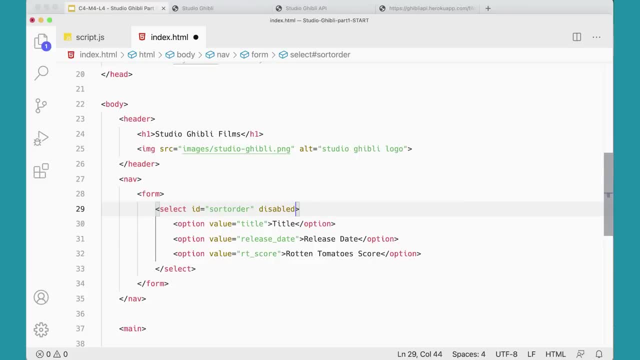 the data has actually loaded. And when you do that it's going to make that sort thing run, which is going to then run the add card function. But the add card function can't do anything because the variable with all the data in it hasn't been filled out yet, because you haven't gotten the data. 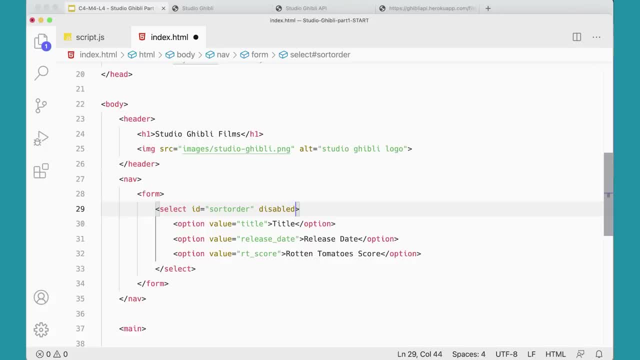 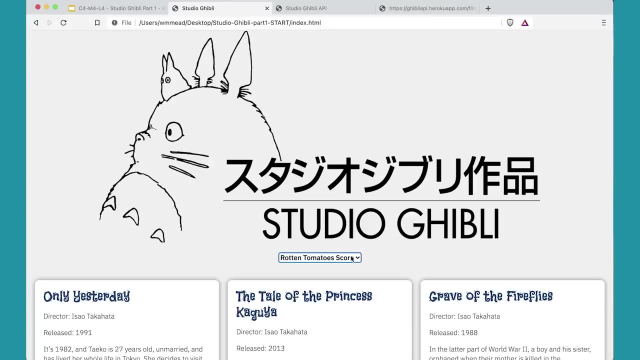 So that would cause problems, That would cause an error and cause some things to happen. I mean, it's it's a lot of work. It's pretty unlikely that somebody could come and actually, you know, try to use this thing before the page initially loads, but it's possible. 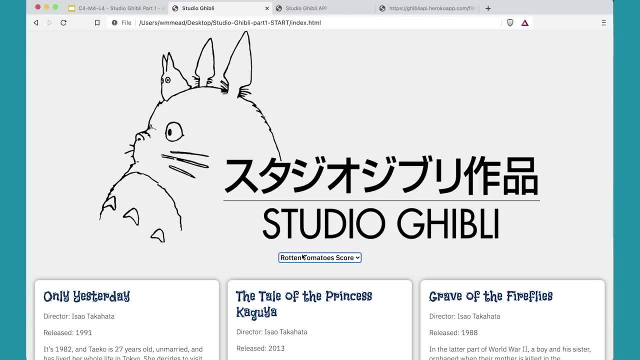 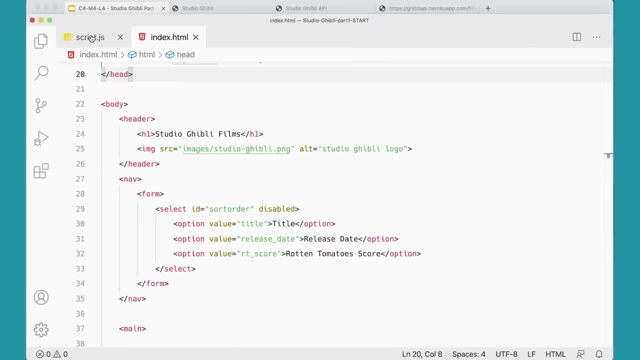 So what we'll do is we're going to have this thing come up, initially disabled and then enable it once we've gotten the data and we know that we have the data, So let's go back. I'm going to save that And go back to our script file here. 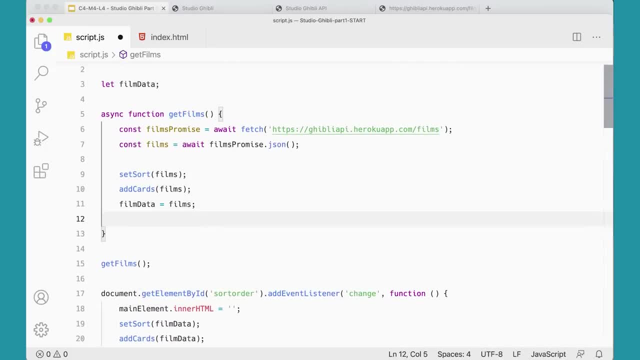 And just at the bottom of our get films function. I'm just going to add one more command here And that's going to document get element by ID. sort order: remove attribute disabled. So that'll remove this attribute disabled as soon as this asynchronously has gotten. 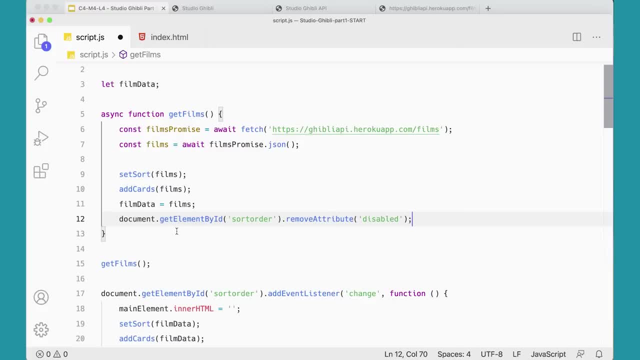 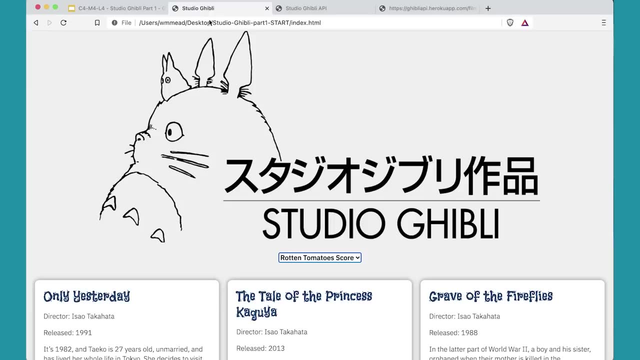 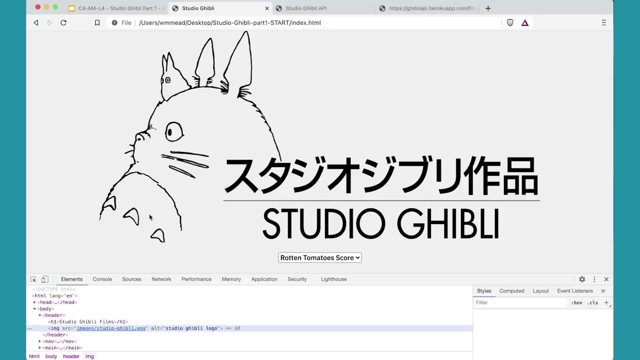 the data, and we know that the data is there. So that kind of cleans that up just a little bit, Okay, So again, you'd have to really kind of push it to see if you could get that to go, but you probably could if you were to go to inspect here. I haven't tried this, it's always a 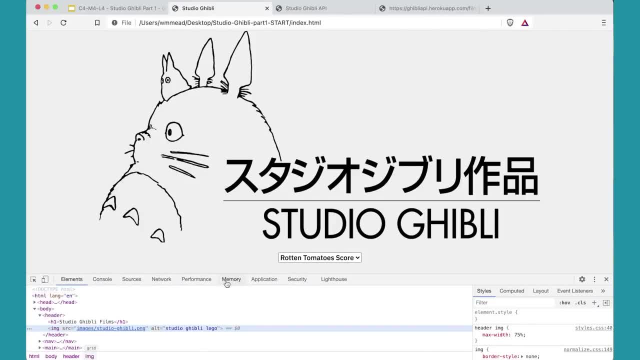 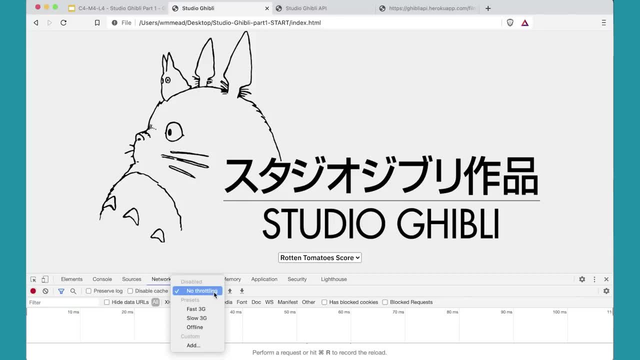 little scary to do this. I haven't actually tried it, but if I go to network and choose a fraudling slow 3G and then refresh- Okay, And then refresh the page, You can see this is disabled until all the data gets in. 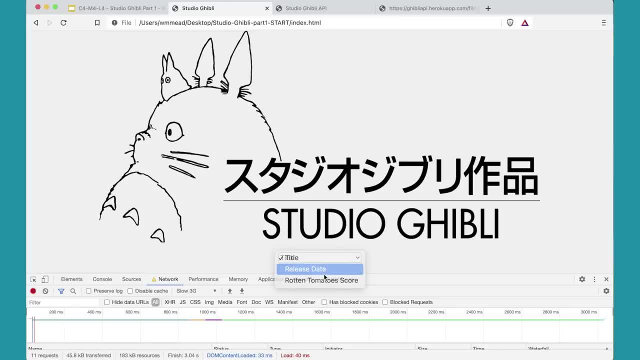 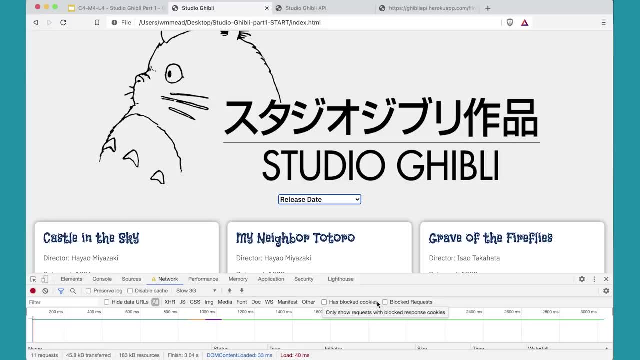 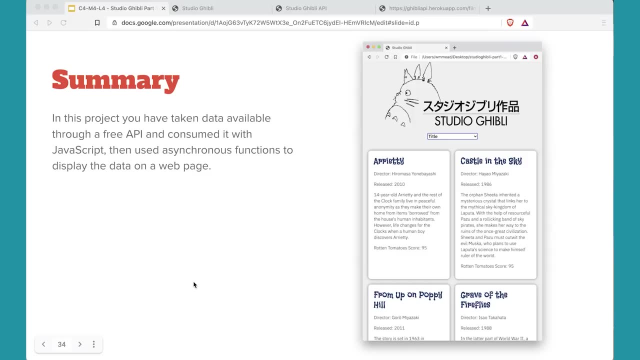 Once the data is in, then it becomes enabled and I can actually sort my films then. So you can kind of see that here by throttling this thing down. it's a nice little feature. In summary, In this project You've taken data available through a free API and consumed it with JavaScript, then used. 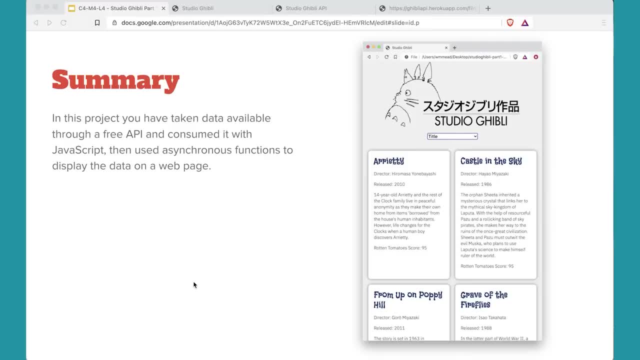 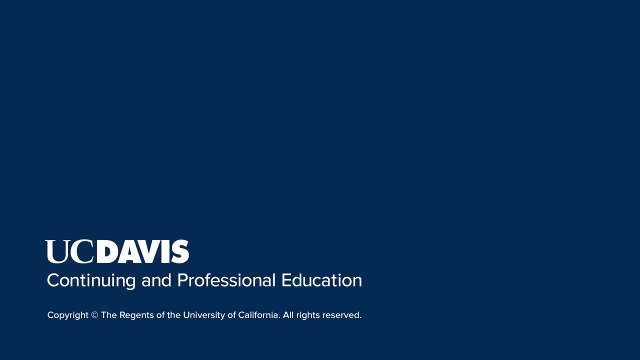 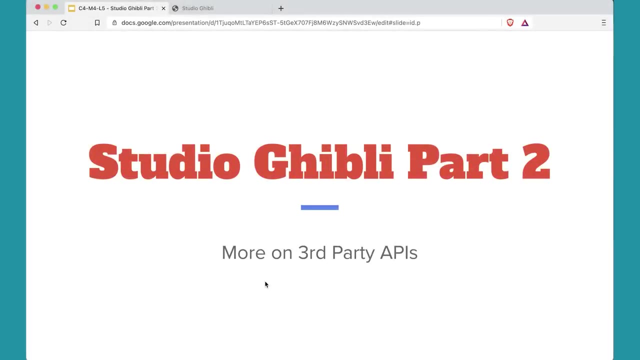 asynchronous functions to display the data on a webpage. That's pretty cool. And then the second part of this project will push this project even further. Studio Ghibli part two: a little bit more on third party APIs and a little bit more practice. 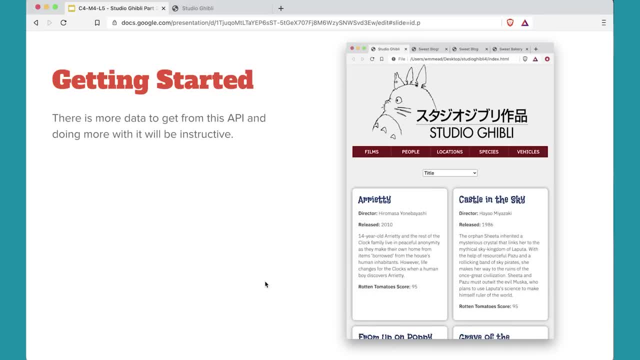 We can get a lot more out of this if we continue working on this project. so let's keep going on it And, to get started, download the new start files that go with this version of the project, because they have some additional HTML and some additional styles that make it easier. 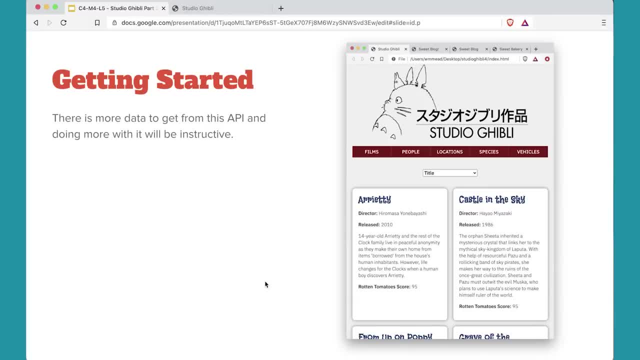 And then, once you've done that, copy over all of the JavaScript under the script file for this, for this version, or you can just replace the script file for this version with the new script file or with the script file from the first version. 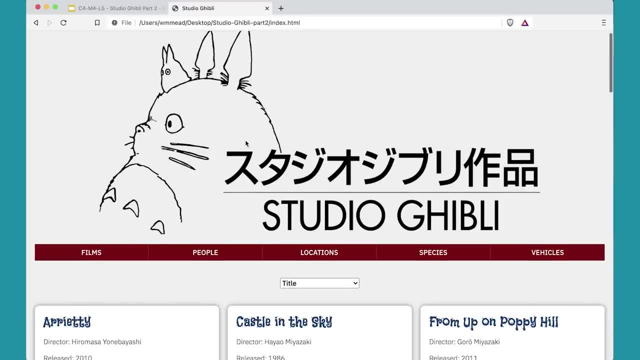 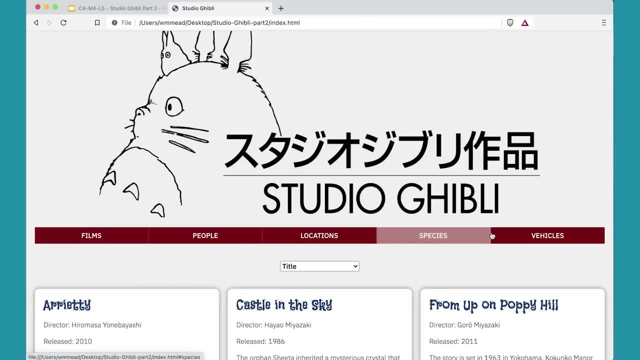 And I've done that over here already, So I have mine coming up and you'll notice. what's different here is, I've got this navigation item here and we're going to create out these different pages because the Studio Ghibli API can not just give us films, but can tell us about the people in the films, the locations. 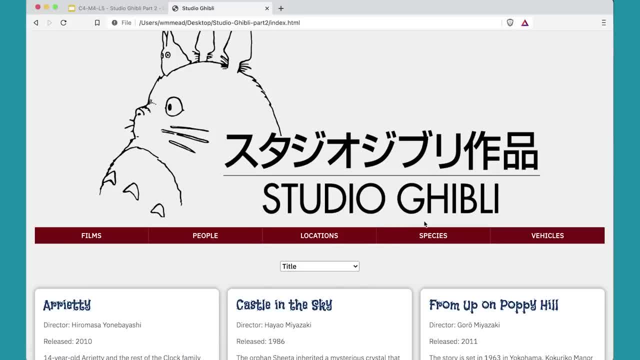 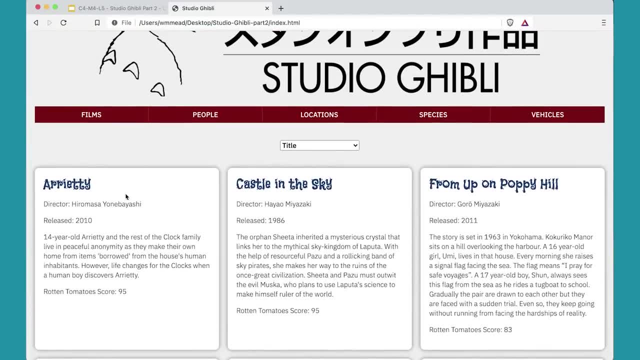 the species and vehicles. Okay, So we're going to build out each of these pages with data from this API in the in this part of the project, But because I've copied over my style, my script as it is so far, all of that is still. 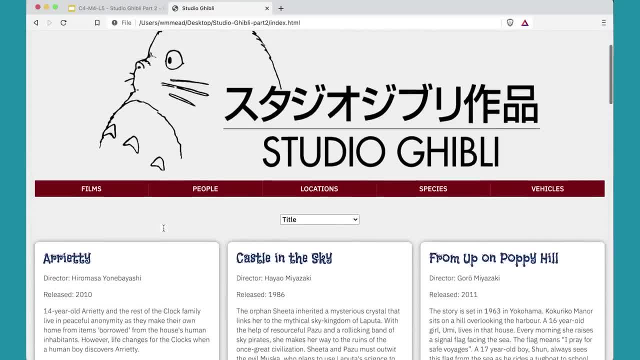 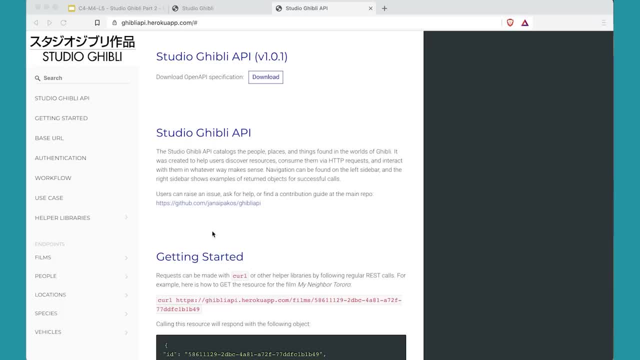 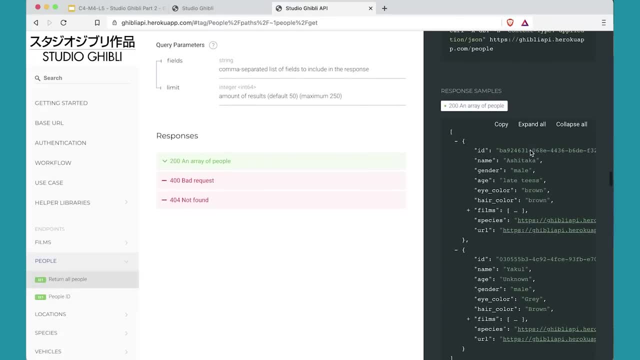 working on the films page and it's pulling up the films just fine. So make sure you do that before you go too far. If you go to the Studio Ghibli API and go down to people here, You'll notice, if you look over here, that the sample data that you get here, at least 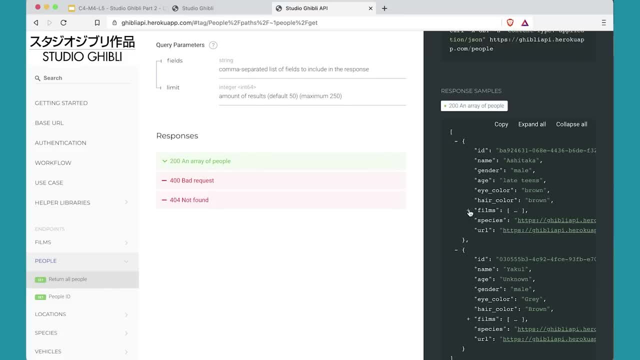 the films. one contains an array and in that array we get at least one film listed, sometimes more films listed, for you know, with links to films there, URLs for films, depending on where those people show up, There might be more. 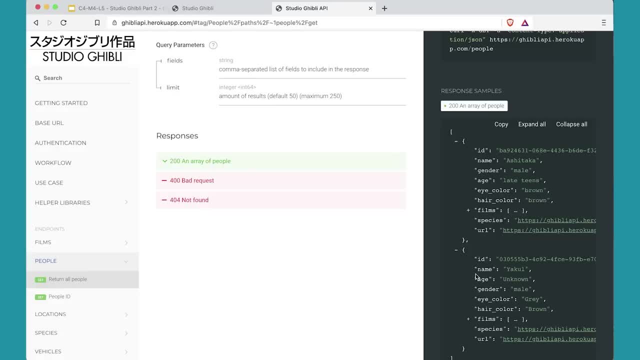 They might show up in more than one place. Okay, So that's kind of interesting. And also you'll notice that some different information is shown here: Name, gender, age, eye color, hair color, that kind of stuff. So that means our create card function is going to have to be different for each page. 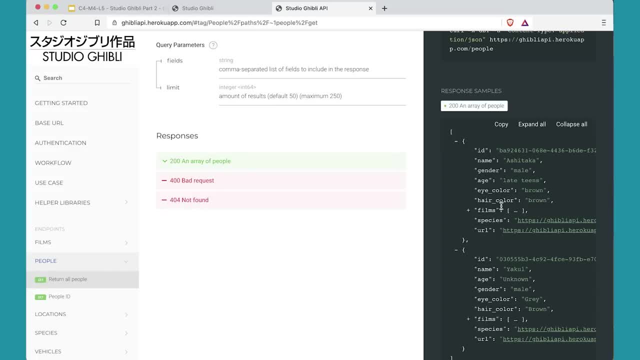 of the site And our current create card function is a little bit cumbersome the way it is, So we're going to change it to use inner HTML to create all the guts of the card instead of using this create element. So we're going to change it to use inner HTML to create the guts of the card. 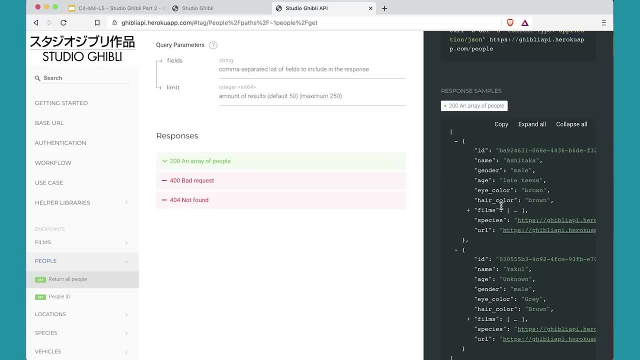 So we're going to do that, But we'll do that in a different way later in the video. So that's kind of interesting And that's the component approach that we did in the first part of this project. So that's kind of fun and should be kind of interesting. 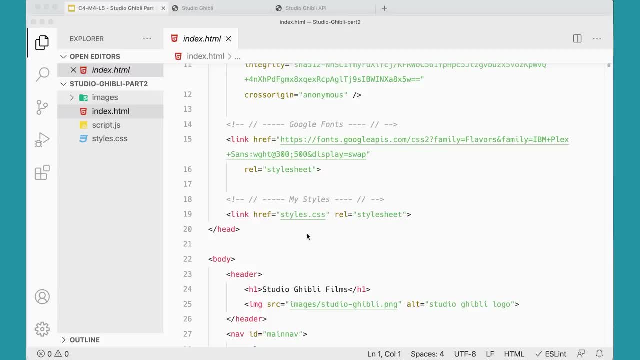 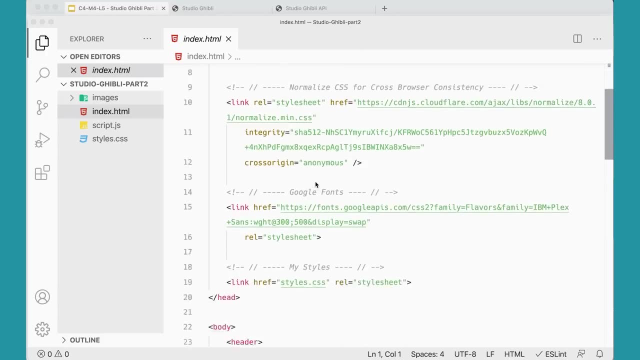 And we'll work on that. next, Coming back to the code editor, make sure you're working on the correct version. I can see up here. it's my part two file here And if you scroll down you can see I've got my main nav here with this unordered list. 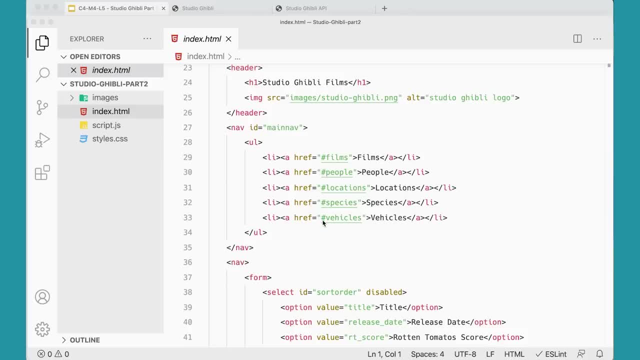 of this navigation in here, So that's pretty helpful. And then, of course, the other thing that we're going to do is we're going to change this page to our own Over here on my script. I'm going to come in here. 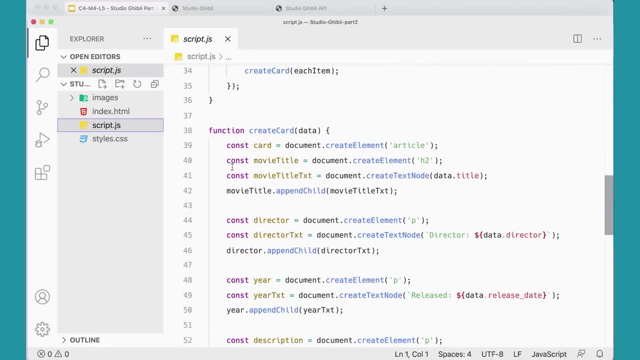 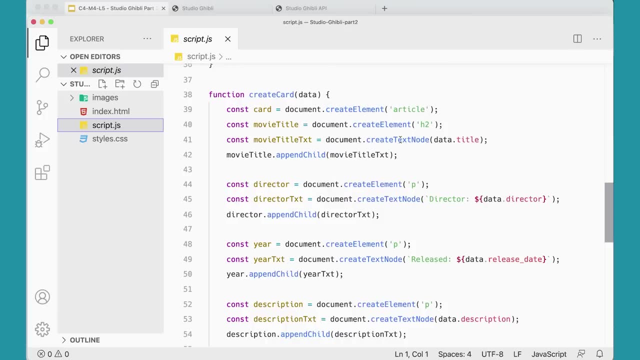 and I'm going to find my create card function And the way we're doing it here is we're creating each of these elements: document create element, create the text node and put the text node in the element. It's really kind of cumbersome. 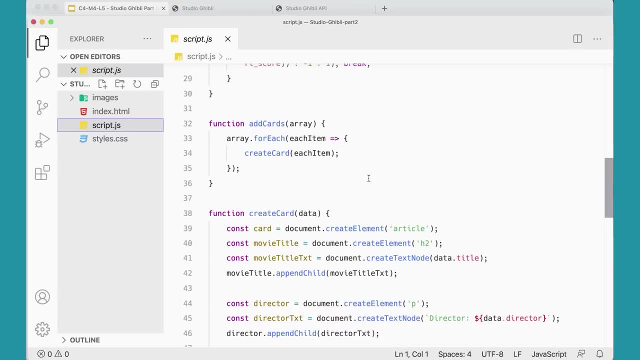 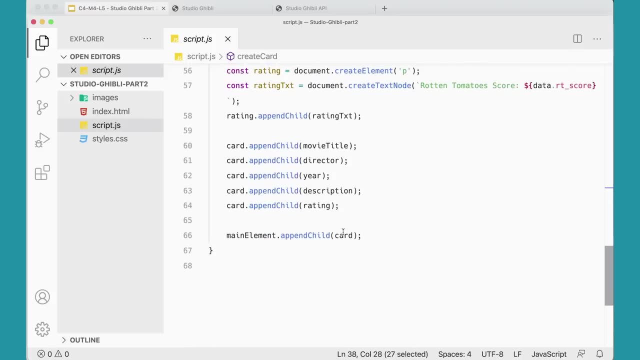 I'm going to replace this whole function, So I can just delete this entire function, starting with here, And I'll hold down shift and go all the way down to here, All of that, and just press delete, Just get rid of it. 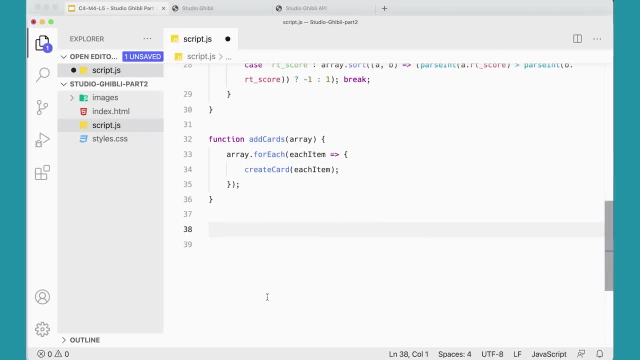 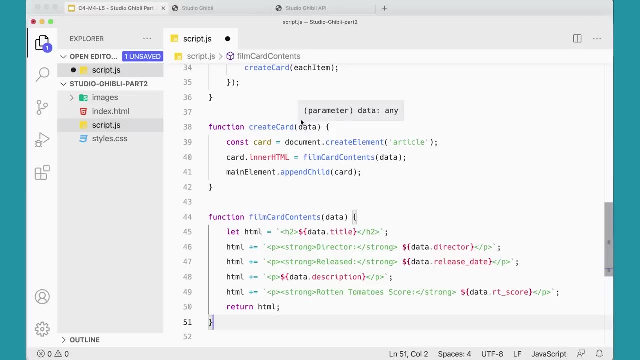 And what am I going to put in place? You're going to have to type this out, but I'm going to paste it in. It's going to be this: It's much shorter, right? So I've got a function here called create card. 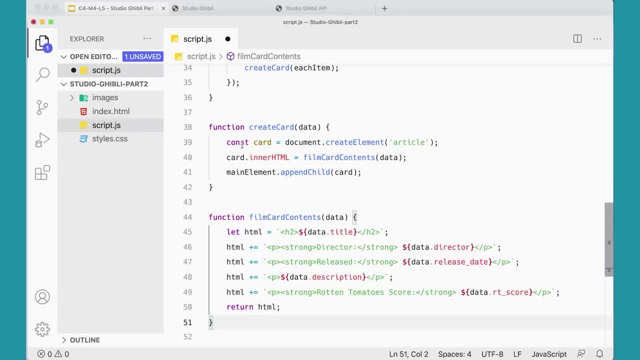 which takes some data, And then I'm going to have a variable called card and that's still going to create the article there And then, and then card inner HTML is going to come from film contents, which brings in data, And then I'm going to append the card to the 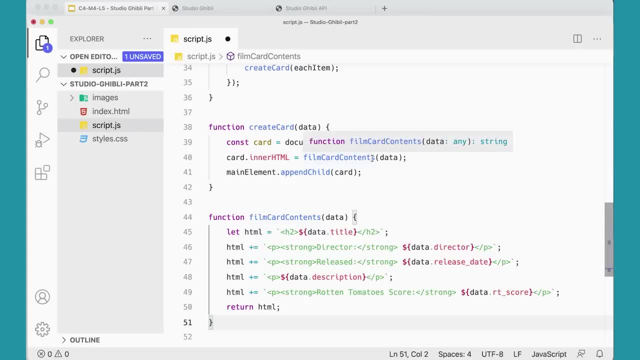 to the main element. So most of the action is going to happen here, down here in film card contents. Again, I'm getting the data and then here I'm just making a variable, let HTML equal and I'm adding the H2. 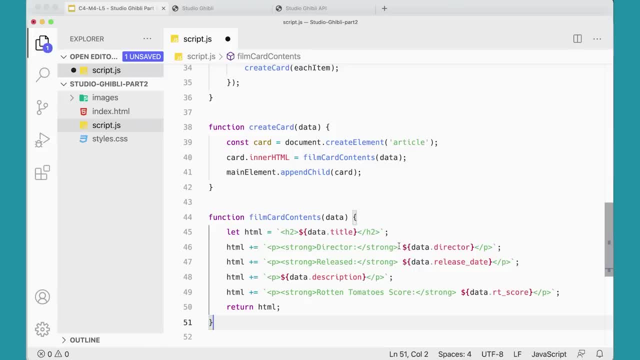 and then plus equals adds to it And I'm adding paragraphs. Notice I was able to add some strong tags in here. I don't know, It's just kind of a little bit nicer, so I can add this all in here and then return that. 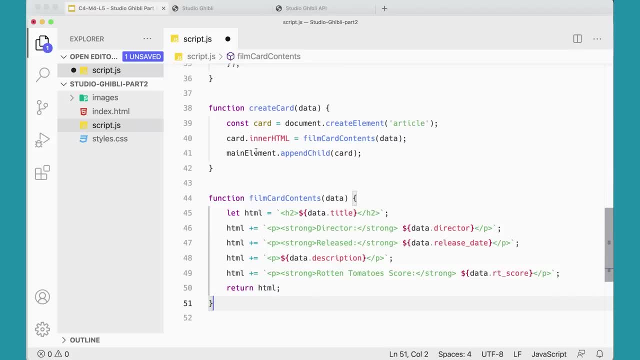 HTML at the end. So this returns HTML. So down here, inner card card, inner HTML film contents data is going to be this returned HTML with all the data that gets put in there. So that's going to be a bit cleaner and a bit easier to. 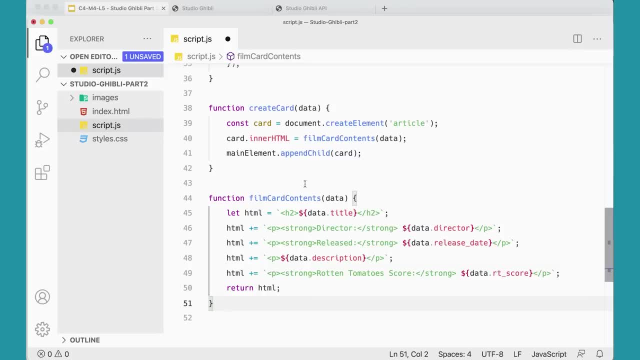 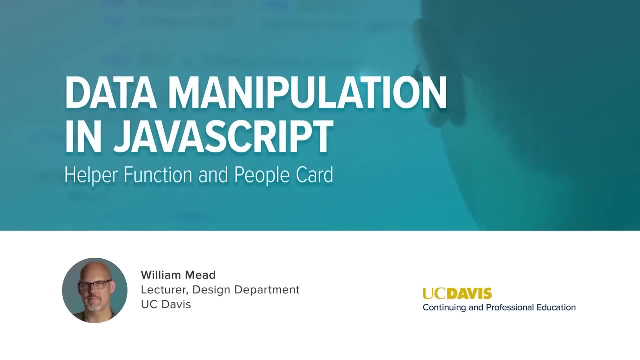 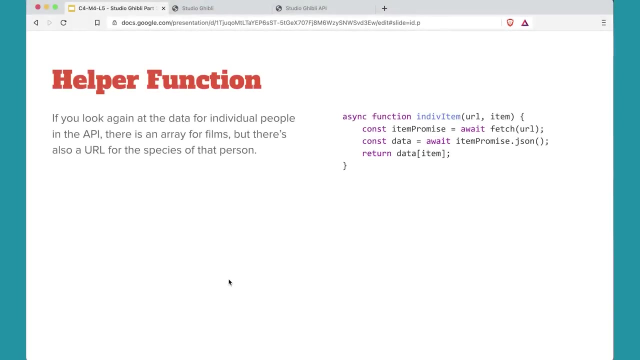 work with, I think, as we move forward, because we're going to have different film card contents for the different pages, But we can use the create card function for all of them. Okay, great, We've updated our create card function. Now we need a little bit of a helper function. 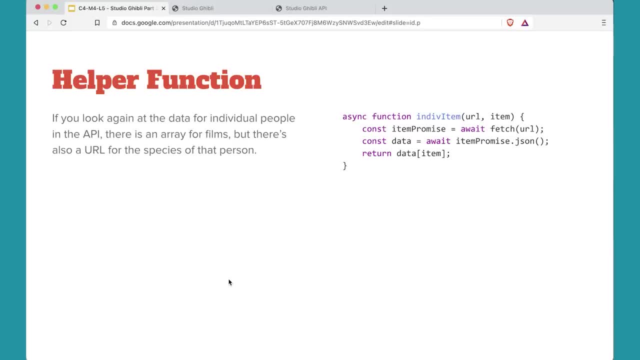 If you look again at the data for individual people in the API, there's an array for films, but there's also a URL for the species for that person. So let's go over and take a look at that really quickly. Down here we've got films and we've got species. 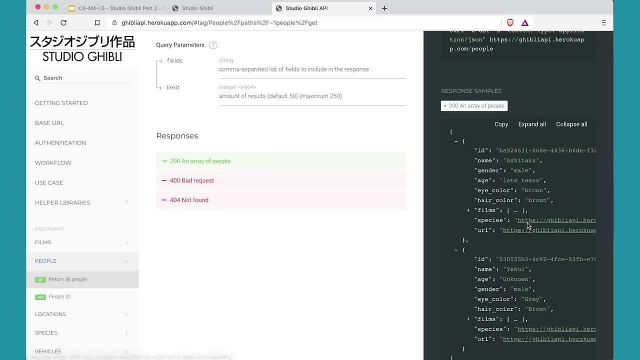 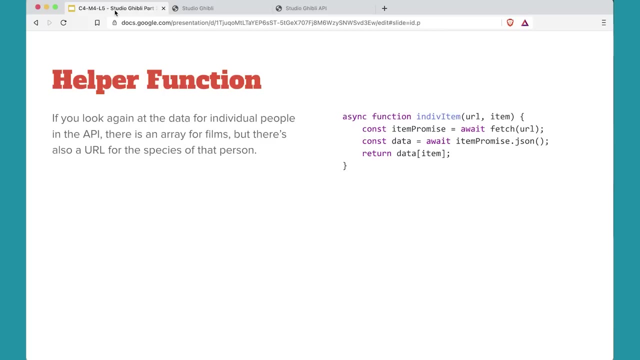 There's a URL there as well, So we need to be able to go into that URL and pull out the species of the person from that URL. And if we want to get the title, we're going to have to use it in a loop, because the title 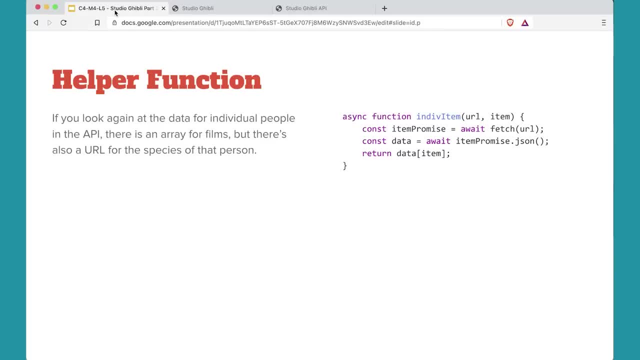 is in an array. So this helper function can be used to go get those URLs. Notice, it's asynchronous: We're going to get an individual item, We're going to pass in a URL the item that we want, and then we go get that item and we return it. 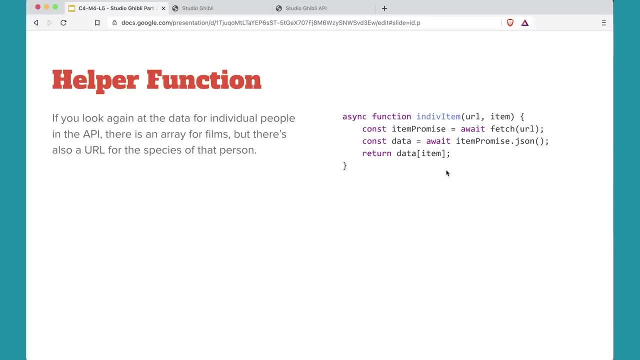 And again, if we're going to use this with the films, we have to use it in a loop in order to get that to work. But this is going to be a helpful little helper function that we can use over and over again in our project. 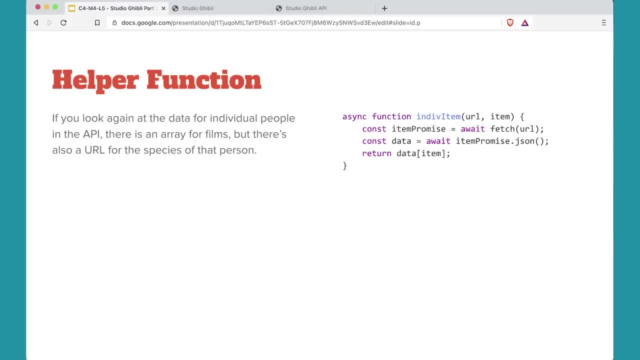 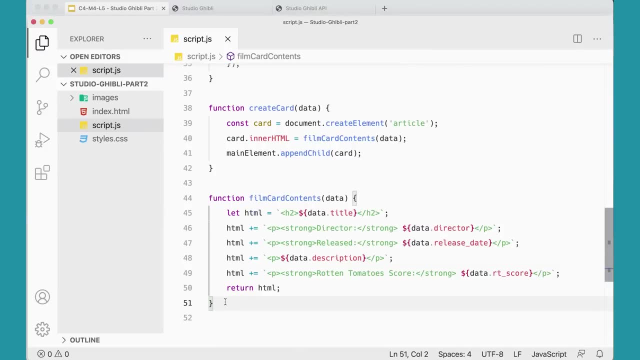 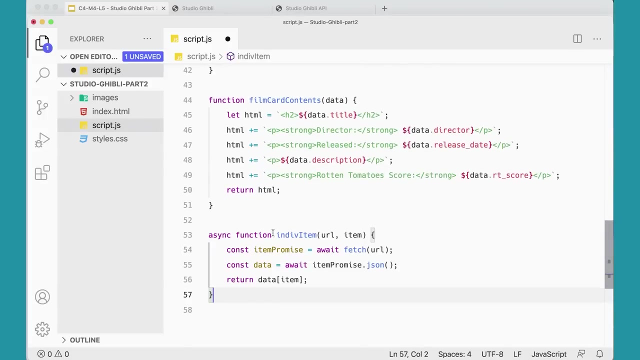 So let's go ahead and add it. I'm going to go over to my code editor and make sure my file is saved And then come down here at the bottom and just add that there. This is kind of a helper function. It can sit at the bottom and we're just going to use it to get individual items. 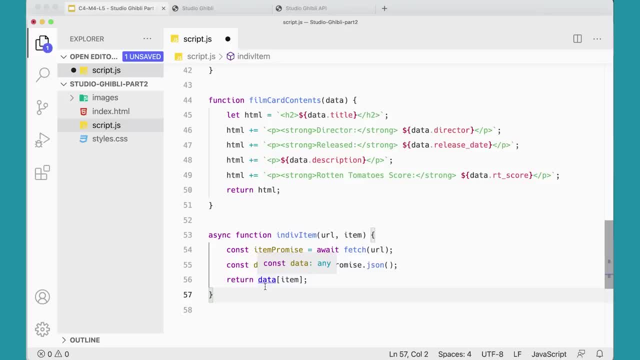 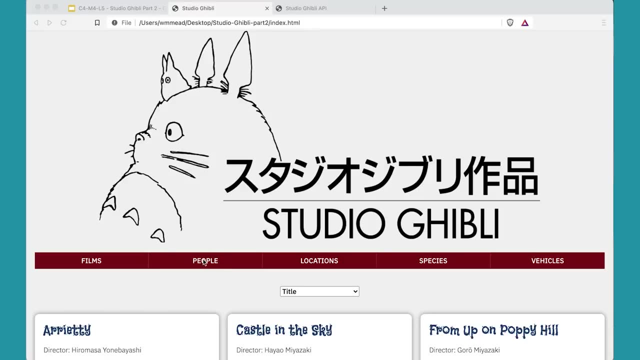 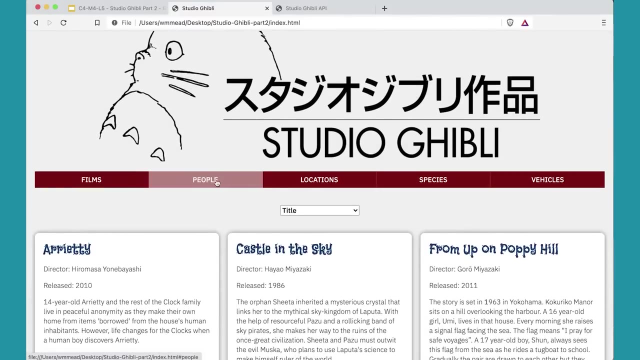 And we'll see how we use this helper function coming up shortly. Switching back to our design, we're going to work on the guts for when someone clicks on the people link here and we get different cards for that for people. So that's what we're working on. 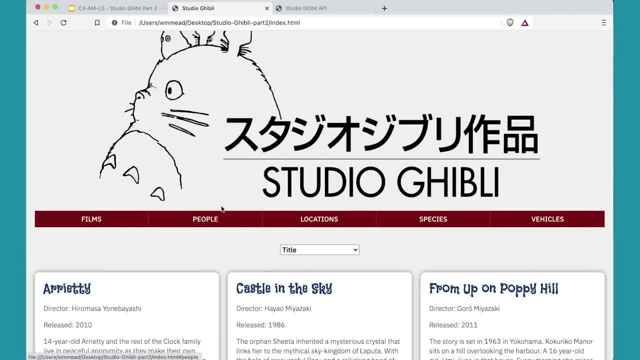 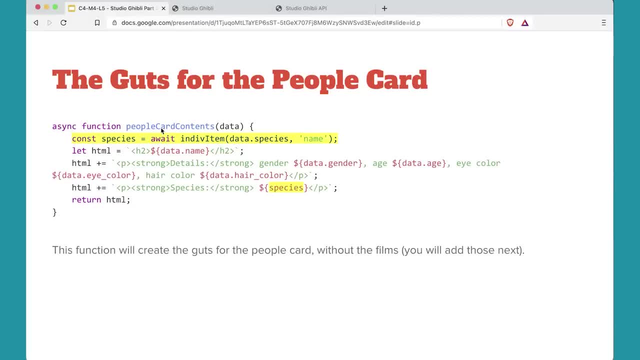 And our data is a little bit different, So we need to create a function that's going to create the guts of those cards. So over here I have a function, an asynchronous function for people card contents. Again, we pass in data and we want to go ahead and add. 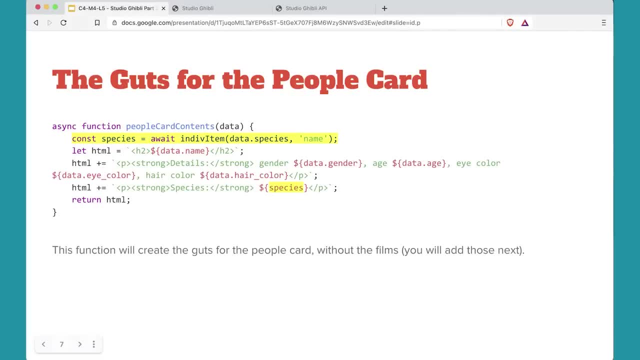 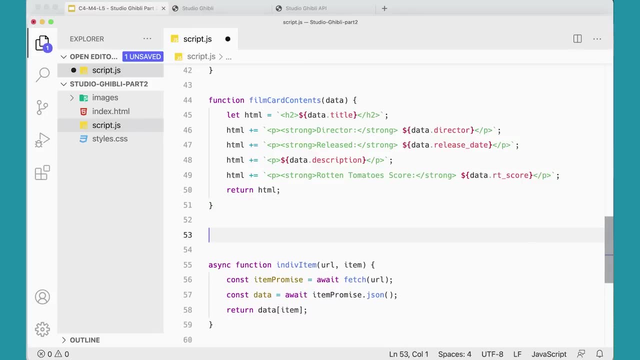 this to our script. So this is what we've created up so far. Coming back to my script file, I'm going to add this function in here. You're going to have to type it, but I'm going to paste it in so you don't have to watch me type it. 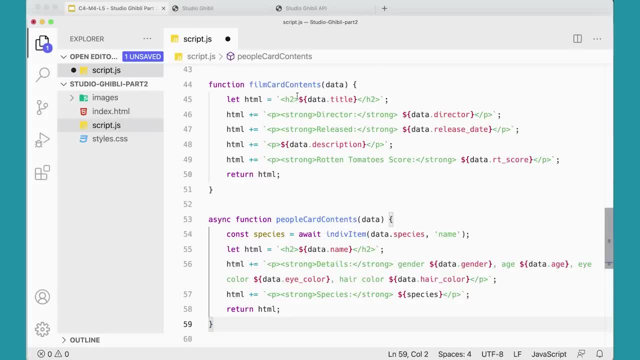 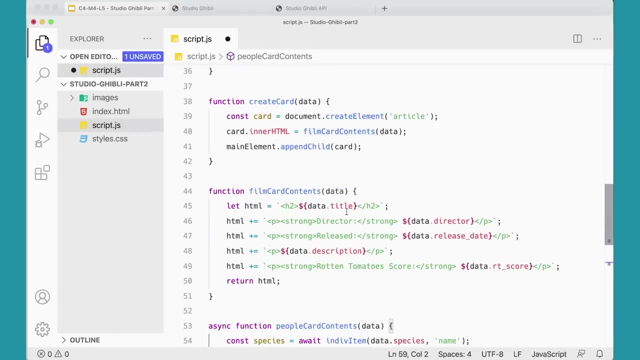 And here. so here we have people card contents. we've got film card contents and people card contents. Up here we're only loading film card contents- We'll fix that in a bit- but down here we've got a new function that's going to generate contents from the people card. 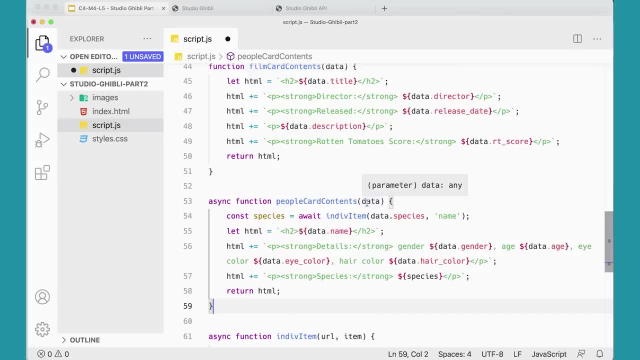 It will get the guts of what we need without the films. We're going to add those next, but notice that since you need to use the use a weight for this individual item, this has to be an async function. Notice this one up here is not an async function. 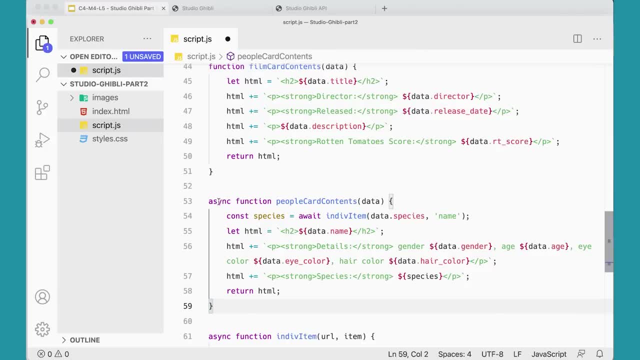 but I can only use a weight here inside of a function that has the async keyword. So that's important to note. Um, and in the individual item function will take the URL for the species from the people data and go retrieve the name of the species from. 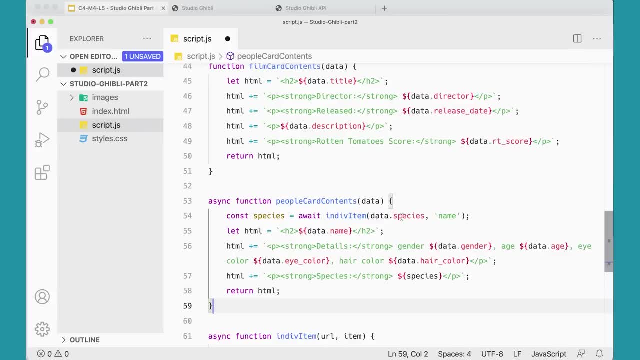 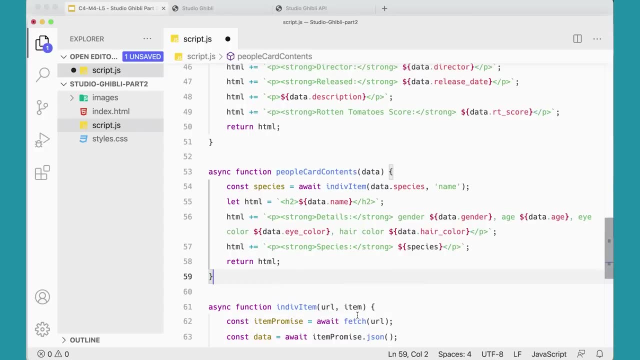 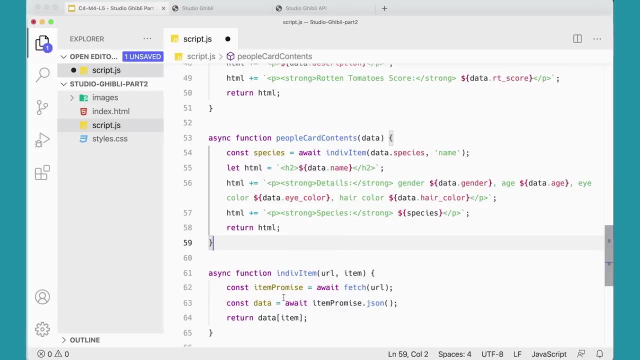 the API. So here I'm running that individual item, data species. I'm passing that in down here for the URL And then the item I want is the name. So it's going to go get that URL, go fetch it and go get the promise JSON data and 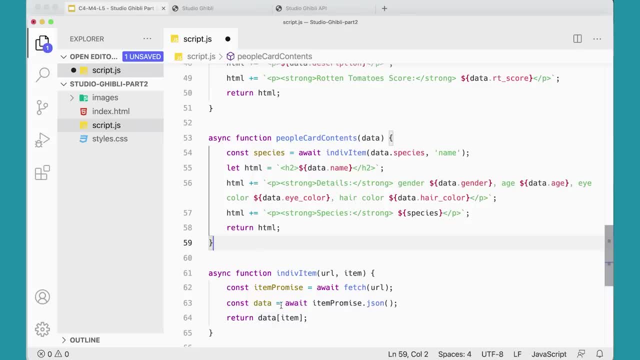 return that thing for that particular item, Data item. So we'll get that particular thing. in this case it's the name, the data species, And what I want is the name from there. but in order for me to use the weight, 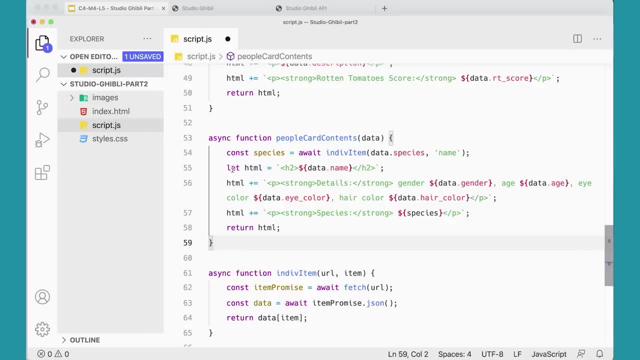 then this has to be an async And then the rest of this is pretty straightforward. I'm making my HTML, I'm putting name and putting all of this stuff in here and returning the HTML. So that's great, That's coming along. 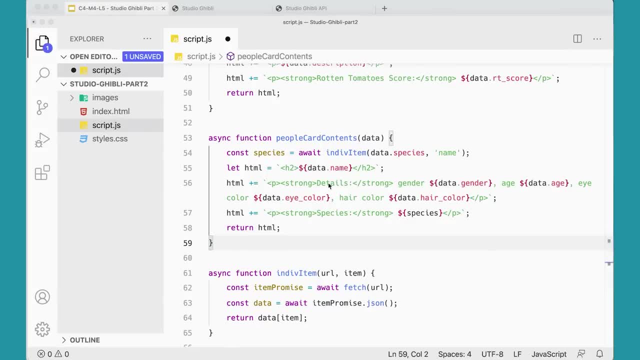 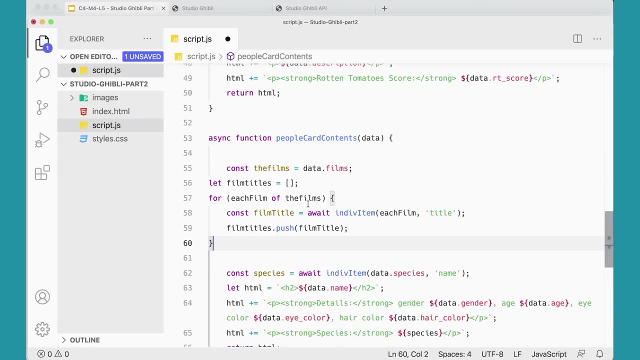 To get the films I need to use. because the films is an array, I need to do this kind of thing but inside of a loop. So I'm going to add to the very top of this function this tab. that in a little bit. 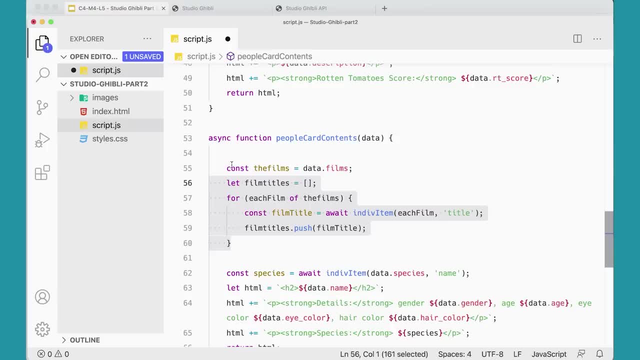 So it looks a little better. There we go, And I'm making a variable: the films data dot film. So that's. this is going to be in An array. that's an array. So I'm going to make a another empty array called film titles. 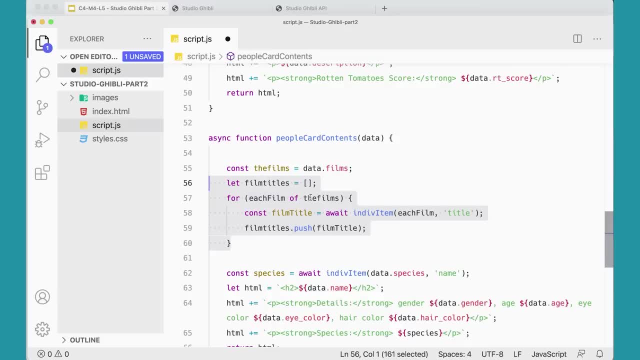 That's just an empty array And then for each film of the films- So this is an array here I'm looping through, using my four of loop- I'm going to make the variable film title and then I go and use my 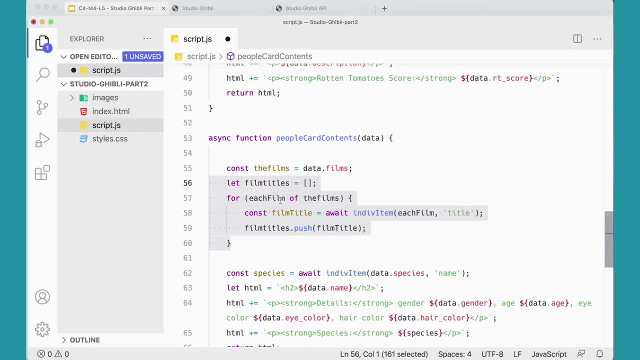 oh wait, I use my helper function to go get that title of the film And then I'm going to push the- uh, the film title up here into this array. I'm going to push into it what I got from an array. 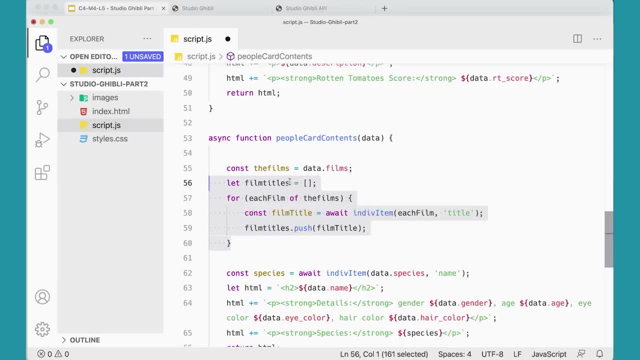 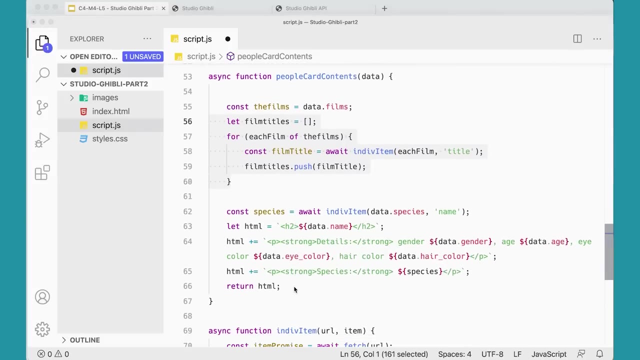 So at the end I have an array here of just film titles and that's just basically a list of film titles there that I can then use. Then I just need to add, I need to add one more piece down here after species down here. 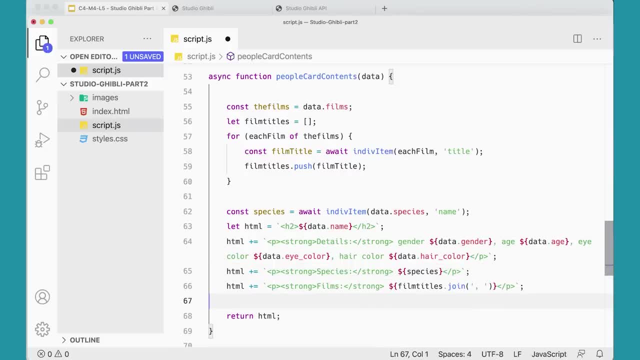 I'm going to add more to my HTML P strong film, strong film titles, And I'm using the join method, which will put a comma and a space after each one of the film titles if there's more than one, so that will do that. 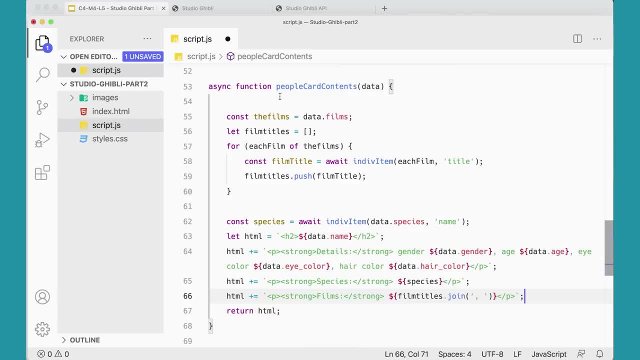 And then it will return that. So this is. this is a little bit hairy with all of these loops in our in our arrays and having to go to the- uh, the API, several times to get data, Cause I'm going to the API to get the films. 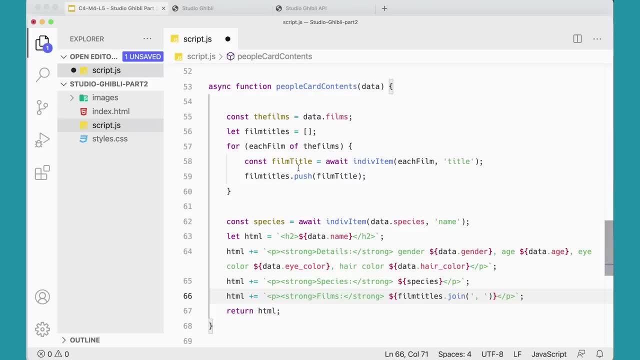 I'm going to the API to get the um, to get all the films and to get the species and then also to get all of this other data as well. So I'm I'm making several trips over there for this. I actually think I want to move the film titles up. 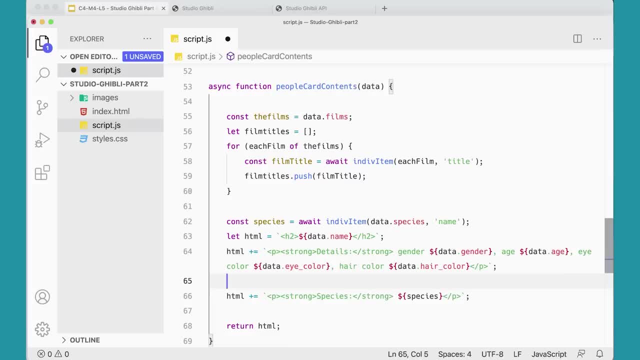 I'm going to put it before the species. I want to leave the species last. I'm going to put it there. It doesn't really matter, You can put it whichever place you want. It just depends on how you want to display it on the. 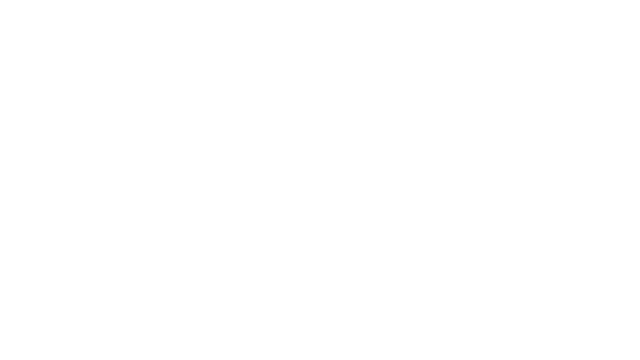 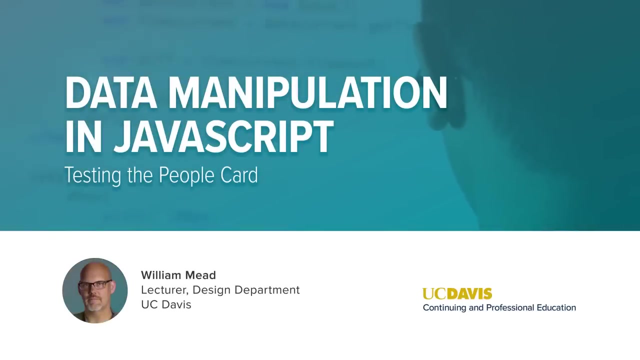 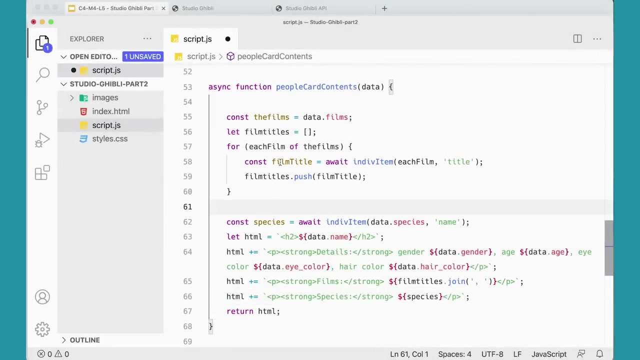 card. I think I'm going to have the film titles first. In the previous video we spent a lot of time creating this people card contents function and working with asynchronous data to get this to go, So hopefully it'll work And now it's time to test it out. 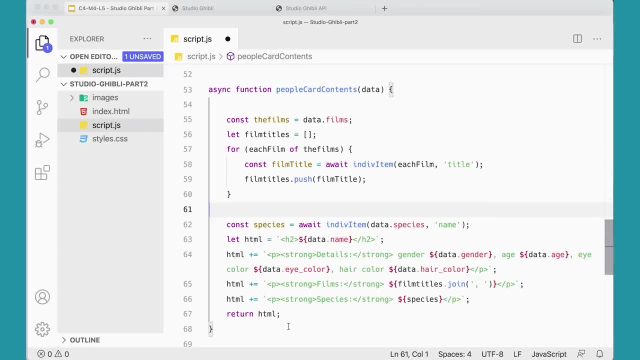 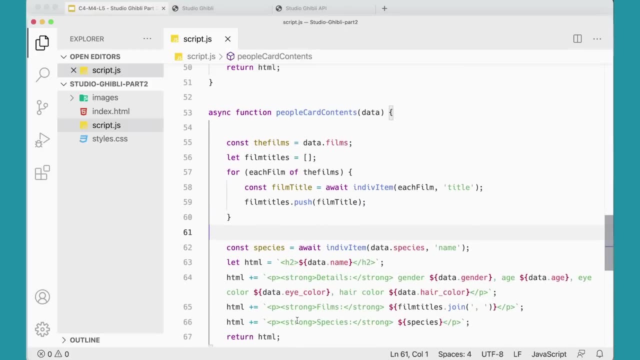 So to test it out, we need to do a few things. We're just going to kind of test it to see if it's working. This is not a finished uh, this is nothing finished yet, but I just want to test it and make sure it's. 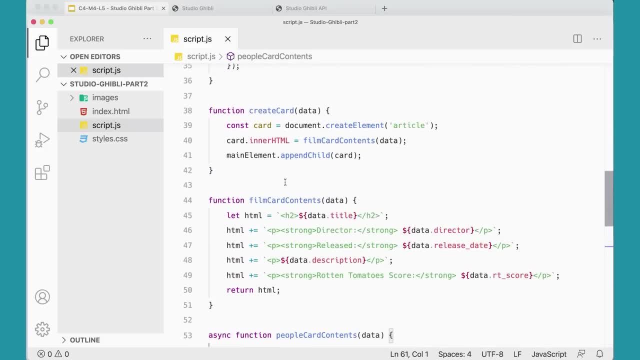 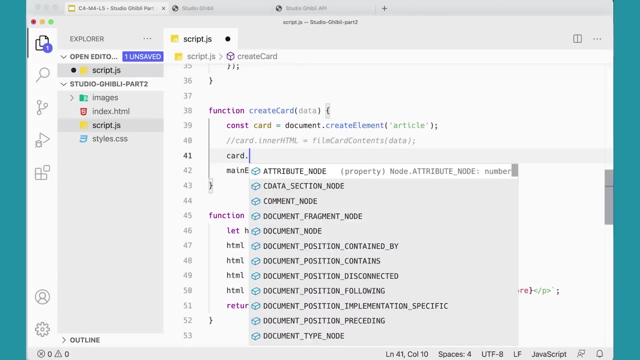 working for now, So I'm going to come up here and where we have card inner HTML film contents data, I'm going to comment That out And instead I'm going to put in here the: this card inner HTML equals people cards. 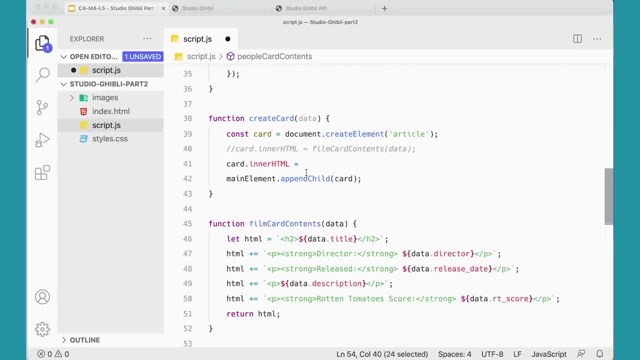 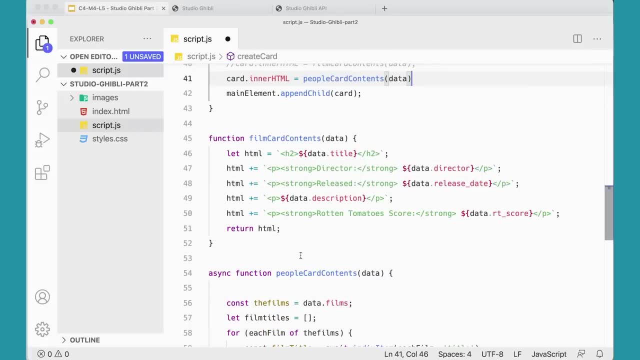 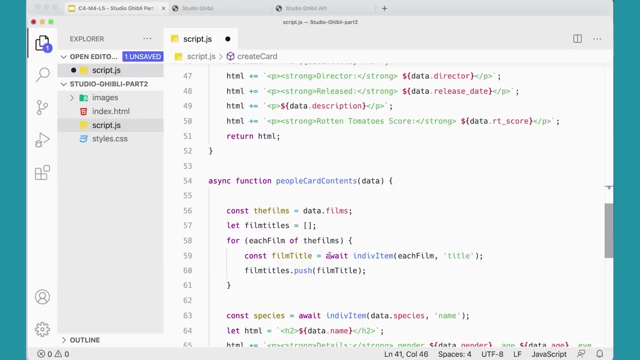 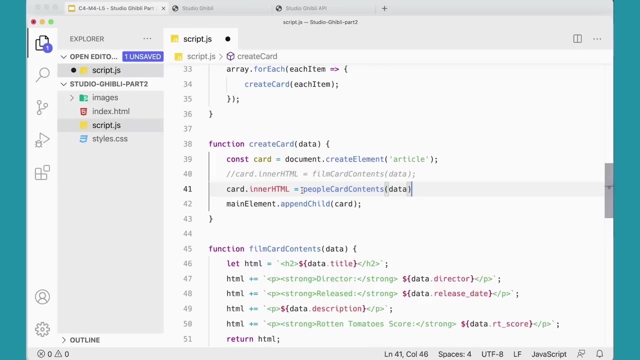 content data that thing instead like that. But because this people contents card data is doing some asynchronous stuff, we've got to wait there. We've got to wait down there. This is an asynchronous function. We have to put a weight here as well. 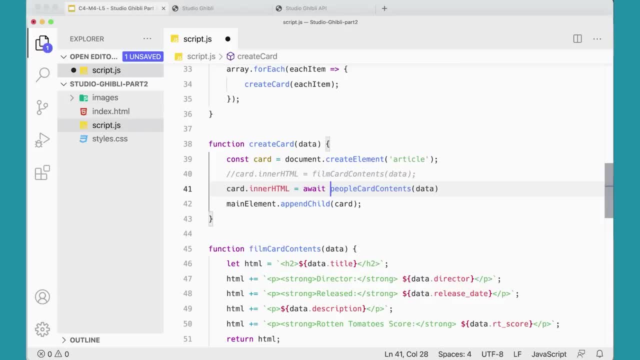 And this is one of the trickiest things about working with asynchronous functions is you is. they tend to look like regular functions, Um, and it's easy to forget this stuff, And, and also because I put a weight here, that means this has to be. 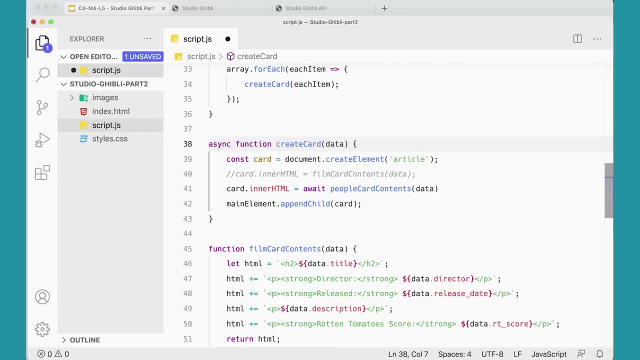 Become an asynchronous function, So I need to add a sync there. All right, So that's one thing that I need to fix in order just to test this. This is just temporary, just to test it- to see if I can get cards of people showing up on. 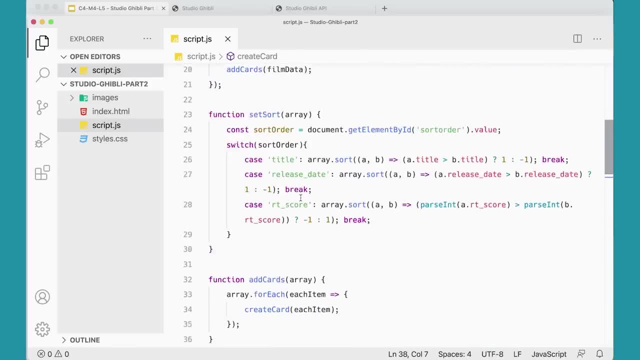 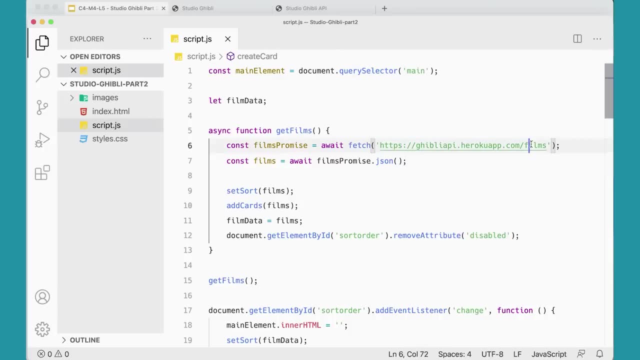 my page And also there are a couple of other things I need to change up here at the top of the page. I'm getting films here And really what I need to get is people. So change films to people, because we're getting people. 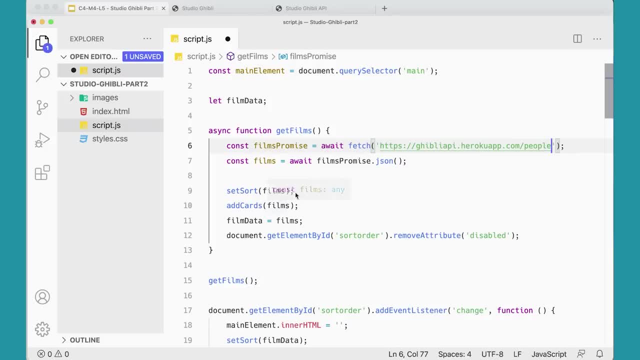 not films. I'm not going to change the names of these variables for right now. We're going to fix all of that later. This is just temporary, to see if it works. Also, you should comment out the set sort, since that's not going to work for. 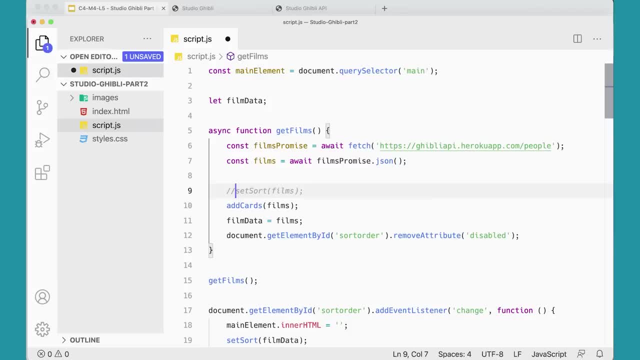 people. It's only going to sort films. And then, while we're at it, I'm going to- I'm going to comment this up, this film data thing out, because we're not putting films in there, We're getting people, So I'm going to comment that out as well. 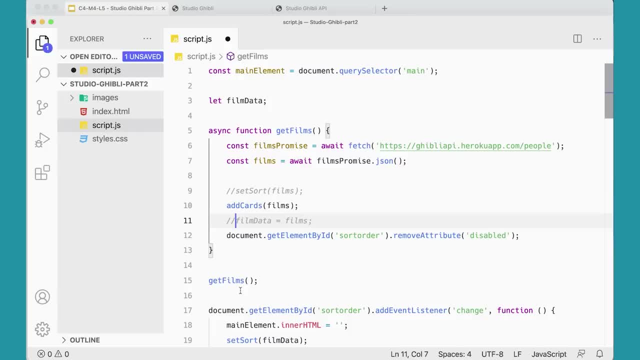 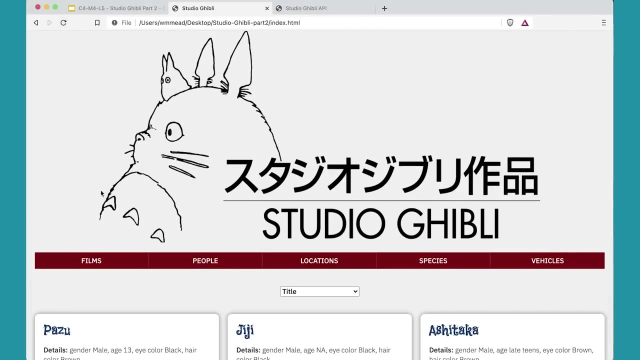 And I think that that's everything I need to do to test this, And hopefully I did everything right and it will work. Let's come back to our browser, make sure that it's all saved, refresh and look at that. I'm getting people and we're getting the films that they're in. 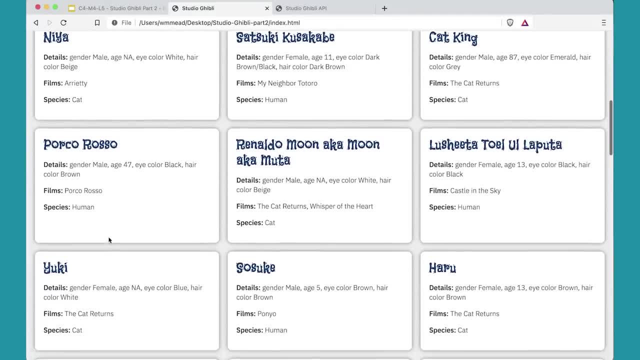 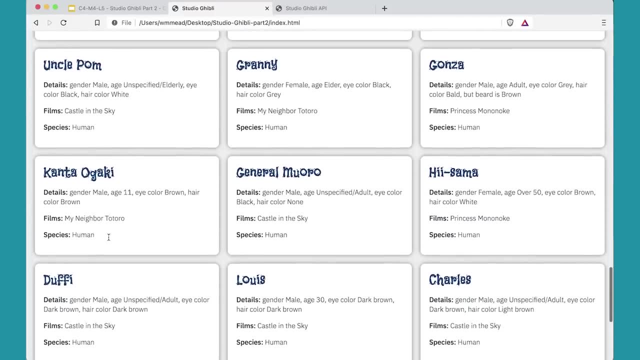 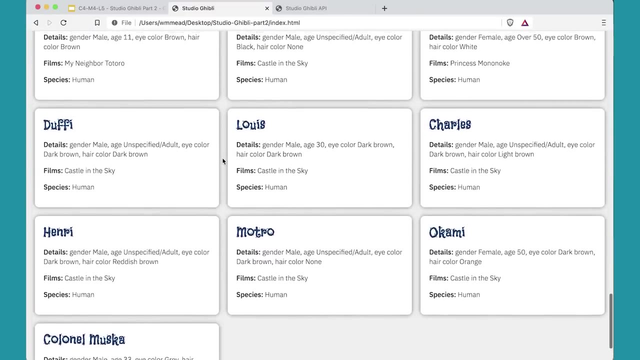 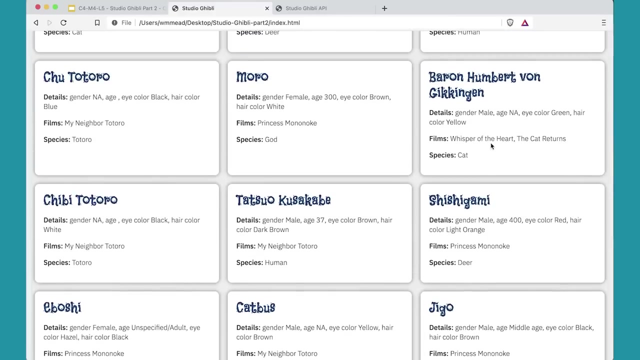 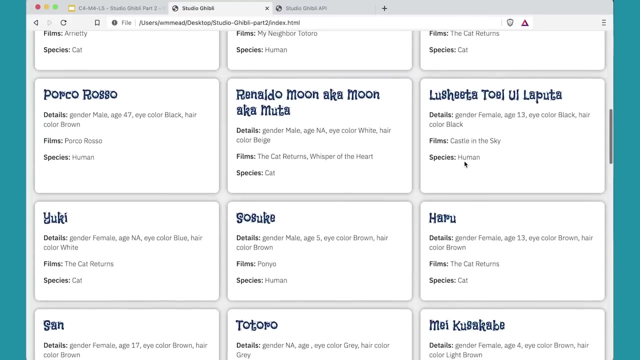 We're getting their species. That's all working, Isn't that awesome. Do I see any that are in multiple films? Here's one, So this one's getting multiple films here. There could be more out. there's another one. That's pretty cool. 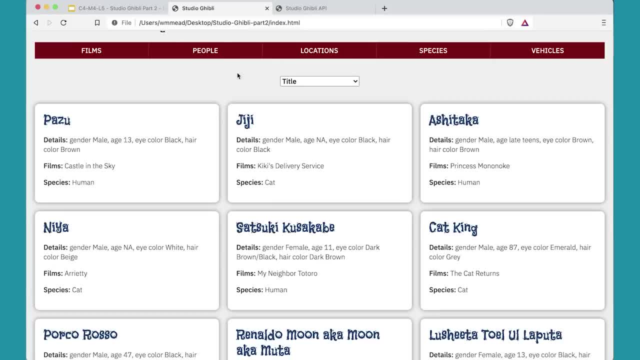 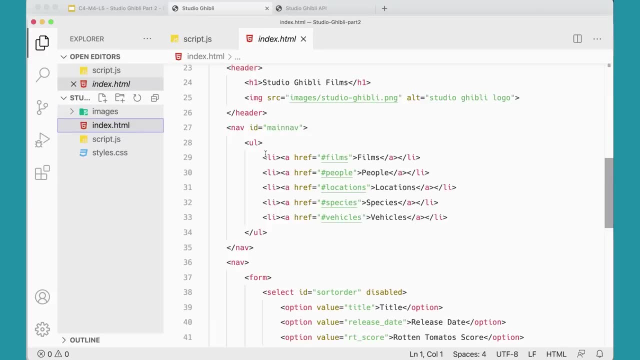 So my film cards are actually working. I just need to make it work now that when you click the people tab and do all of that, switching back to the code editor, look at the HTML file. you'll notice up here. here's my navigation. 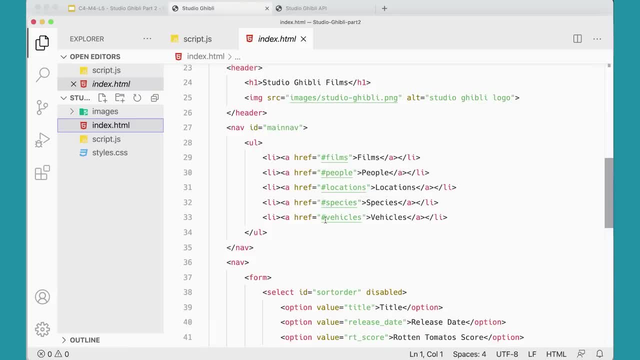 I'm linking to pound films down: people, pound location, pound species, pound vehicles. So these aren't going to be actual pages. There aren't going to be separate HTML files over here for these different pages. Instead, we're just going to fill out the page that we have indexed at HTML with the: 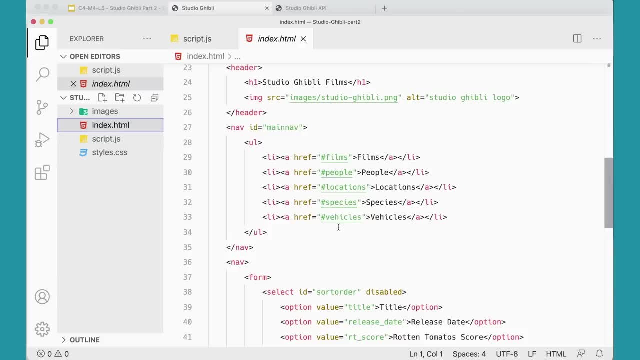 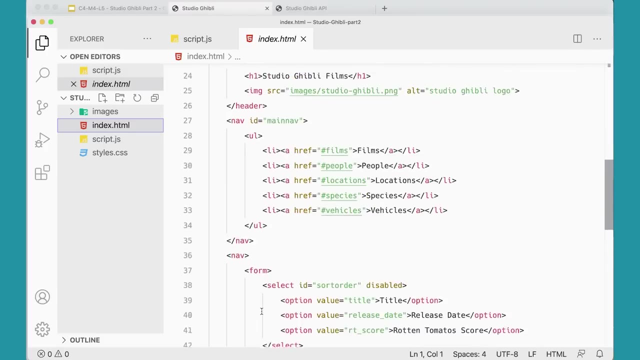 correct cards, depending on which link people click or users click. So so we don't have to make a whole bunch of HTML files in order to do this. We'll just change the guts of this one inside of our main element down here. That's empty, based on which one people click. 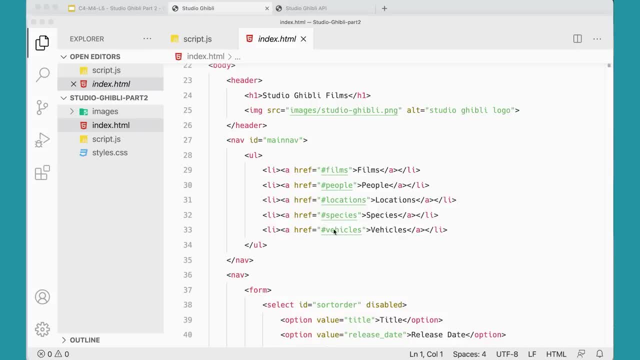 The other thing to note about this list here is that these names in here are actually also the names of all of the endpoints that we have for our API, So we can get films, people, location, species and vehicles If you go over to the API. 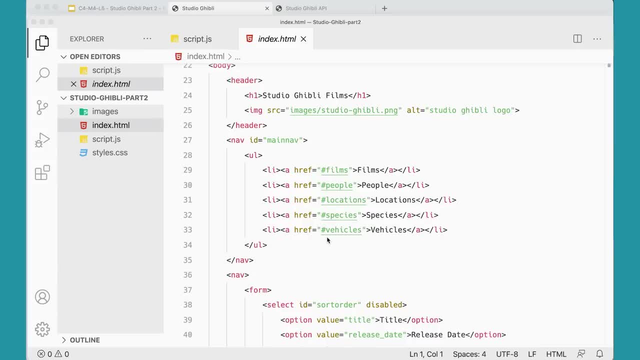 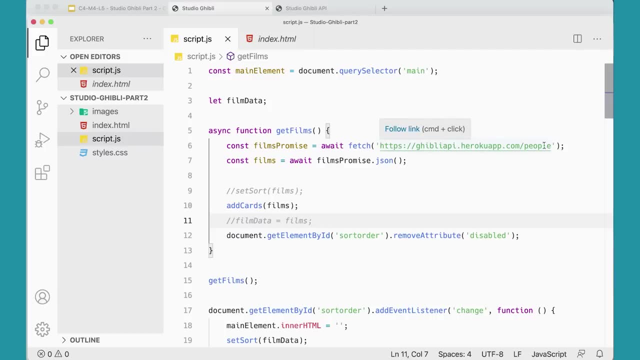 that's the, that's the main, the main names of these endpoints, minus the hashtag. So you, you saw that over here in the script file, where I just change this from films to people, or we can do vehicles, species and all that stuff as well, there as well. 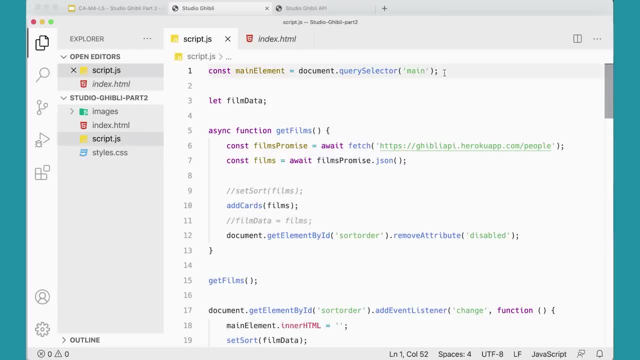 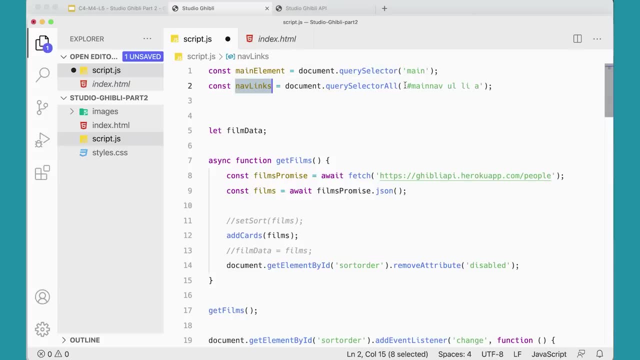 So what I need to add here up at the top of my page here is: I want to get all of those anchor tags, So I'm going to have nav links, document query selector, all main nav, UL, LIA that will come over here and gather all of these. 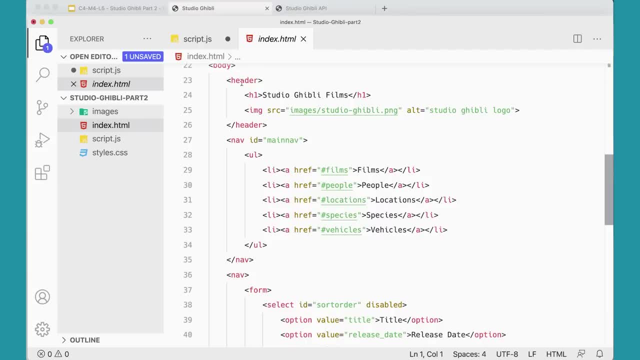 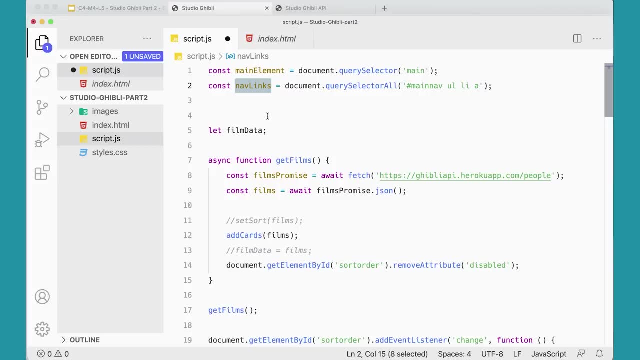 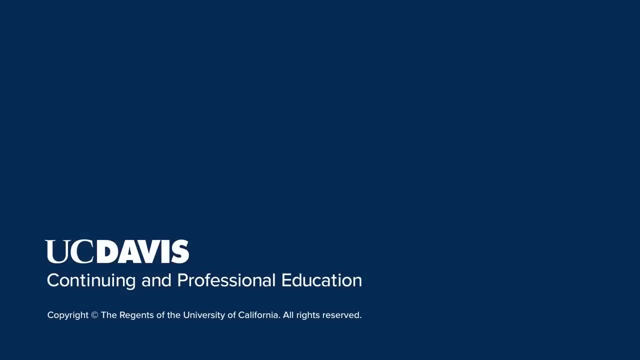 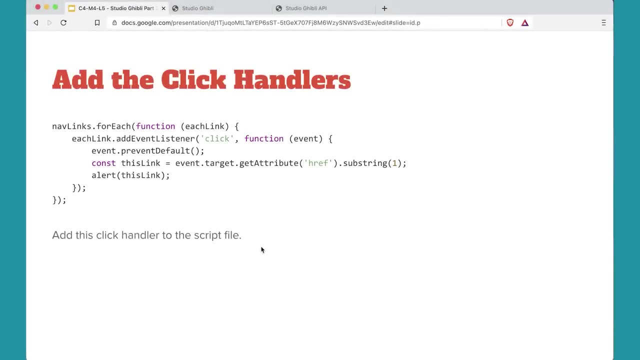 anchor tags here and put them into this variable nav links that I can then access. So I can access ultimately those URLs and, and, and change my, change my page based on which link is clicked When a user clicks on one of those nav links up. 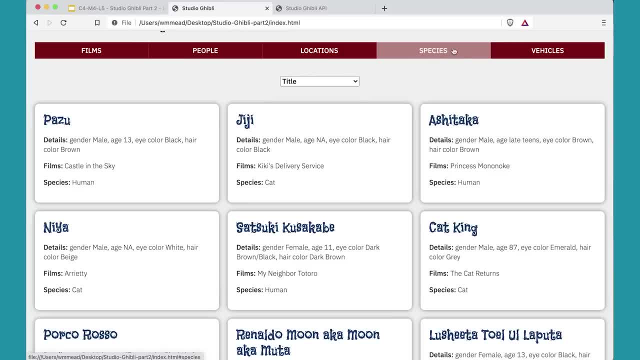 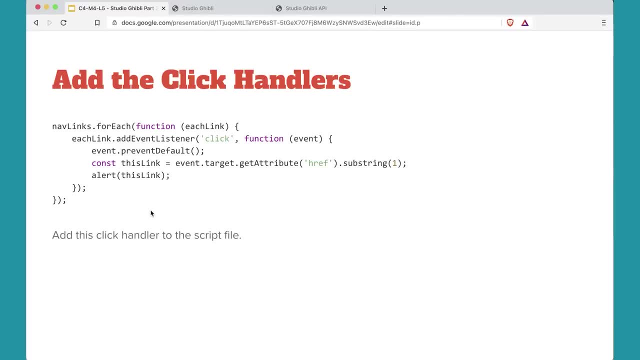 here at the top of my page is here. I need to know which one they've clicked and I need to be able to get the correct data. So I'm going to add a click handler to my script that's going to go through and grab each of those. 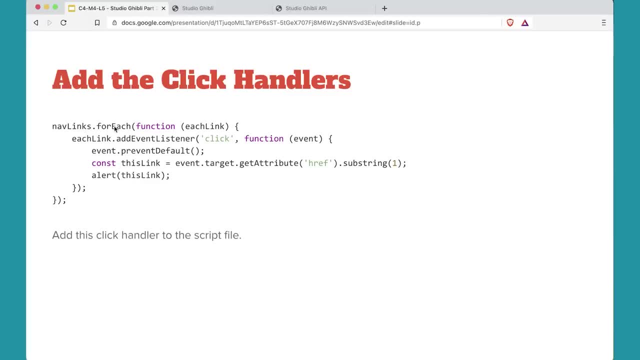 So this click handler goes through those nav links for each one, each link, and adds an event handler on it that adds a click that prevents the default behavior. So there'll be no reloading of the page. And then I'm going to get a variable called this link. 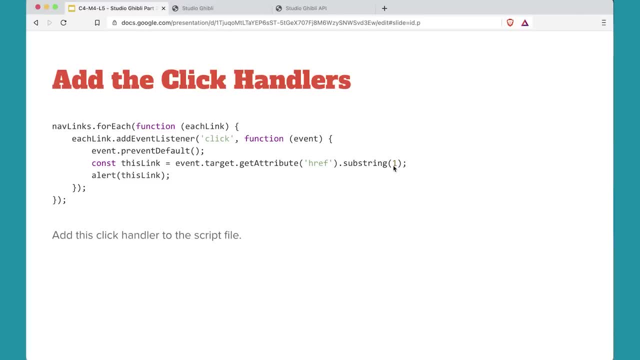 which is event target, get attribute href substring one. So that's going to lop off that pound sign at the beginning. So if you click on people, you'll just get people, not pound people. If you click on vehicles, you'll get vehicles. 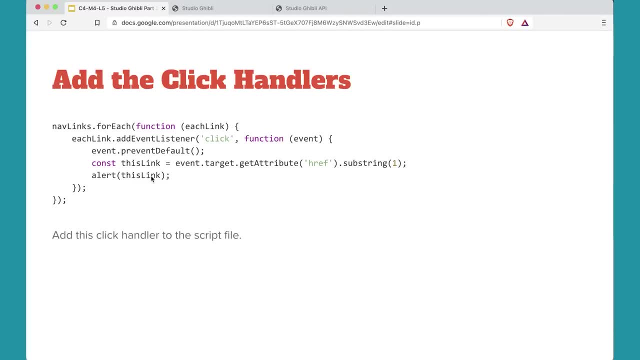 not pound vehicles, And then we'll alert this out, just to see that it's actually working. So let's go ahead and add this to our page. We can put it near the other, the event handler, but it doesn't really matter where on the script that it goes. 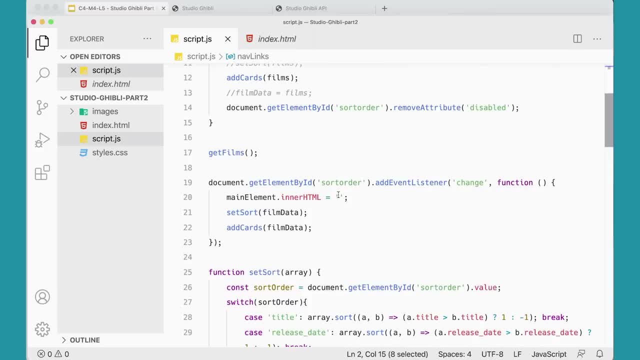 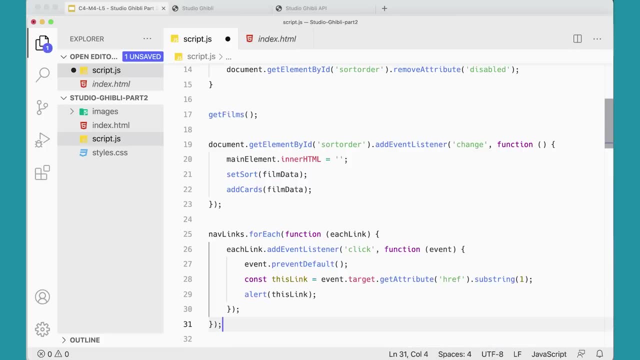 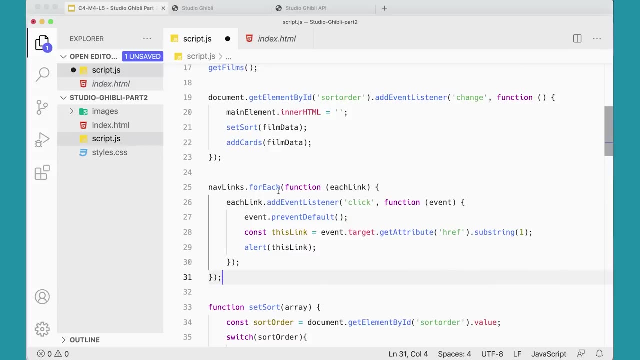 but it's kind of nice to keep these things together. So I have an event handler here for the sort order, So I'm going to add this one here as well, There, Okay, You're going to have to type it out. I've pasted it in so that you don't have to sit. 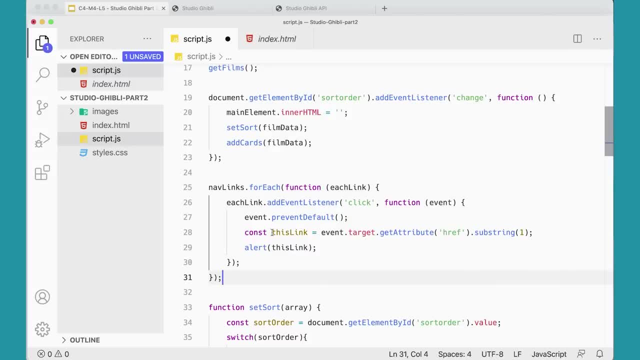 and watch me type it and make my spelling mistakes, but I've typed it before so I don't need to type it again. All right, So you'll have to type that out and save that, And when you have that all in there. 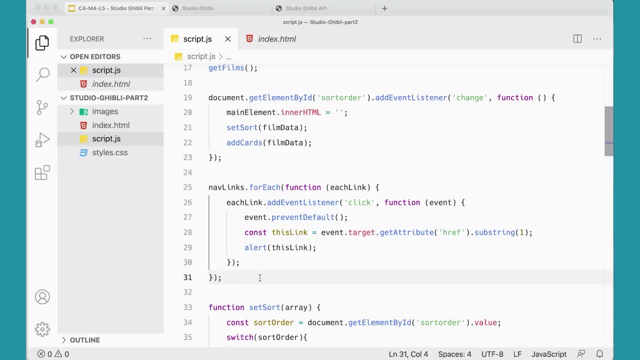 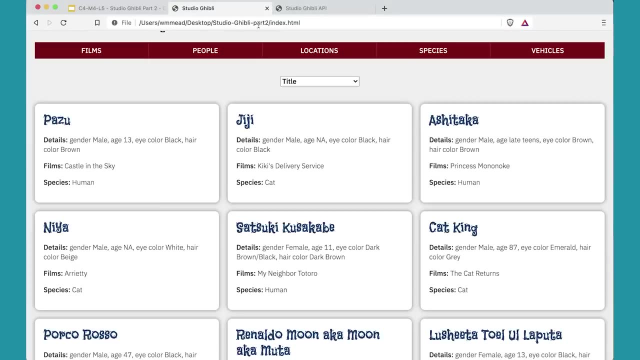 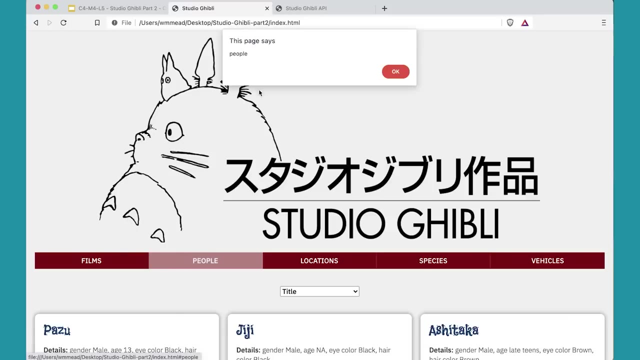 you can pause this video until you have that in place and then come over and test it and see what you get. I'm going to refresh And when I click people, I get an alert that says people. and I click locations, I get an alert that says: 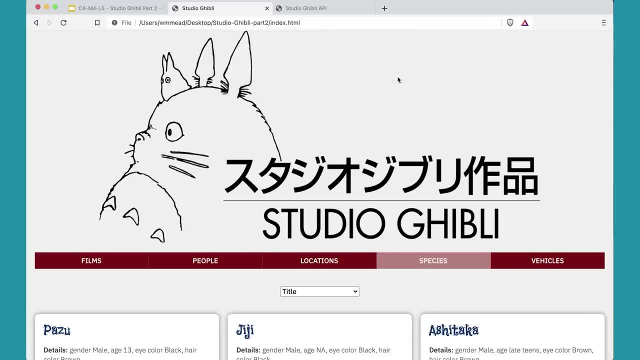 I'm going to get people and I click locations. When I click species, I get an alert that says species, Same for vehicles and same for films. So I can use this piece of data that I'm getting to get the correct data from the API. 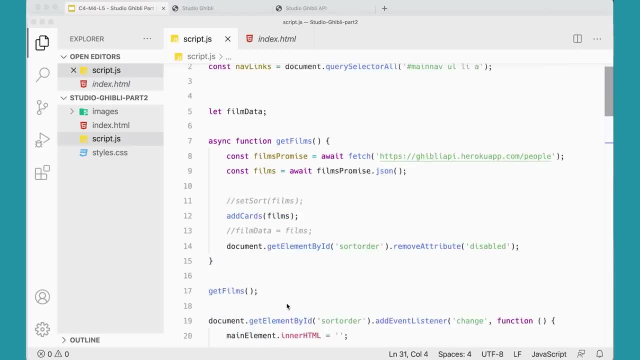 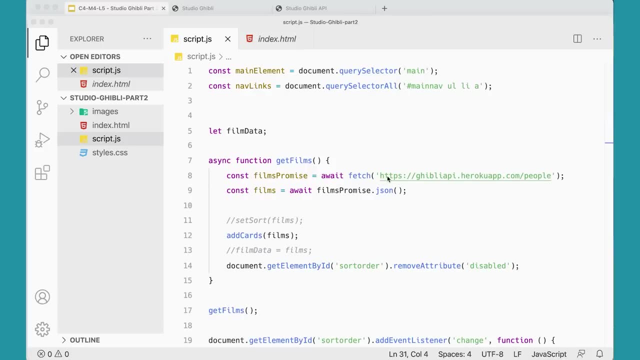 Coming back to the code editor, you'll notice up here that this get films. I have this URL hard baked into this get films thing, but here I'm not getting films, I'm getting people. So that seems kind of dumb And it seems kind of dumb to have it hard baked in here. 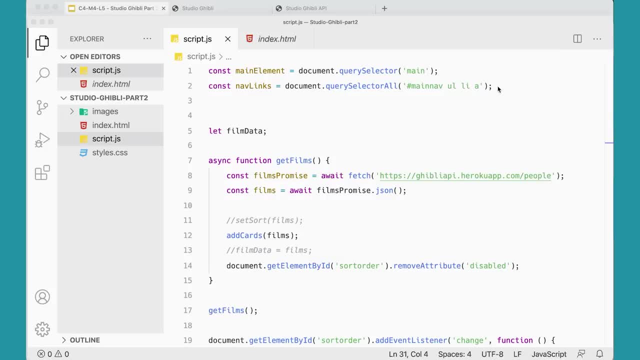 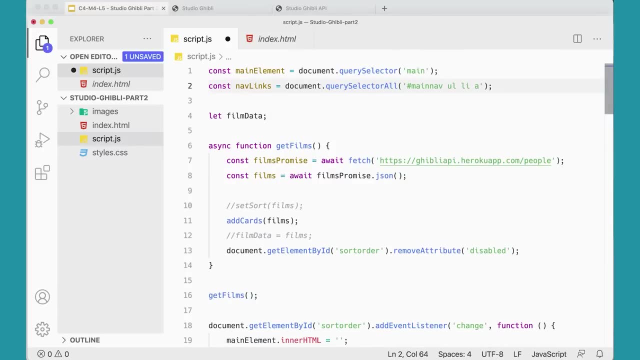 So I'm going to add a couple more variables up here at the top of my script so they can go with the. those are those things. Let's put them with the film data. I'm going to stick them here. I'm going to paste them in. 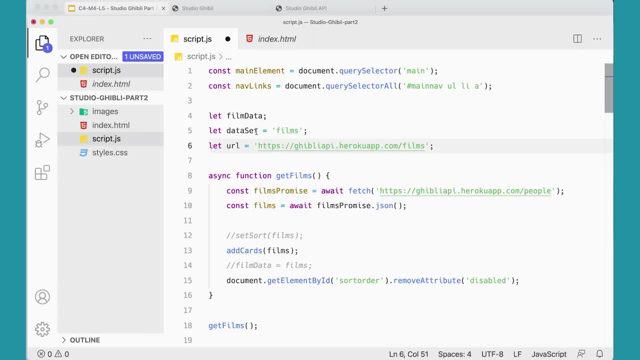 but you can. you'll have to type them. So data set is initially going to be set to films, but when you click on people it should get changed to people And then I've got the URL which is initially set to films. 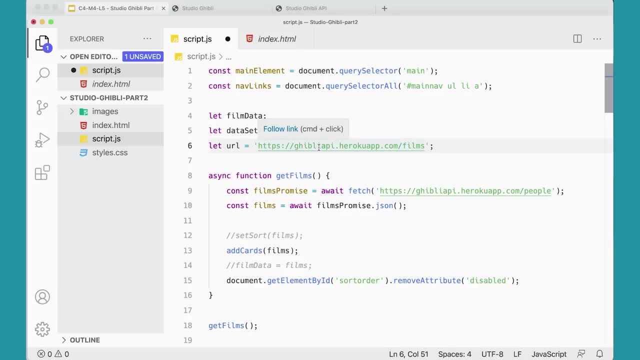 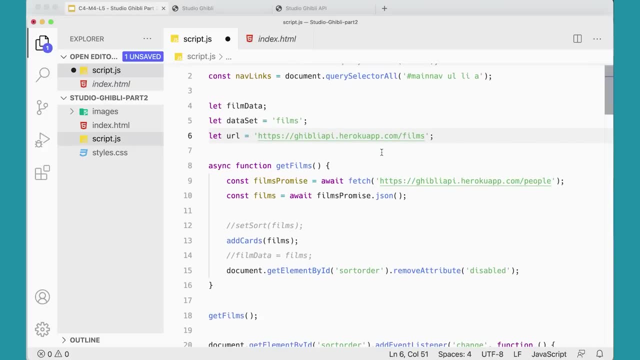 But again, when you click on people, we're going to need to change that as well. So now what I need to do is I need to: here's your challenge. This is: this is a great micro challenge for you to see if you can do this. 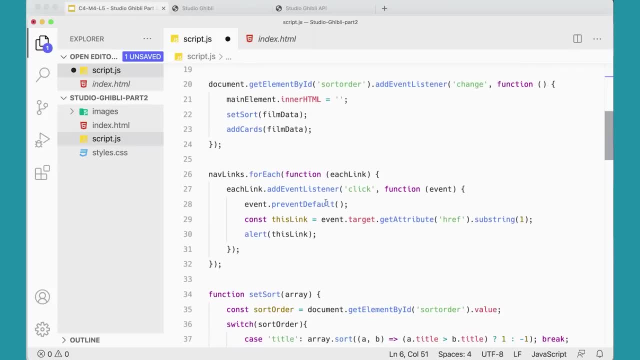 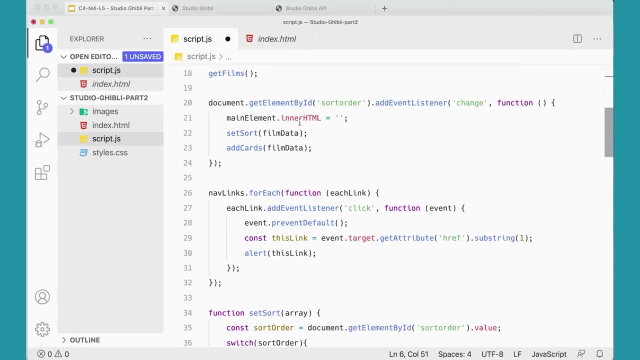 Down here in this click handler. when you click on these, on these links, I need to change these two variables that I've just set up here. So if you click on films, this link is going to be films. I need to change the film. 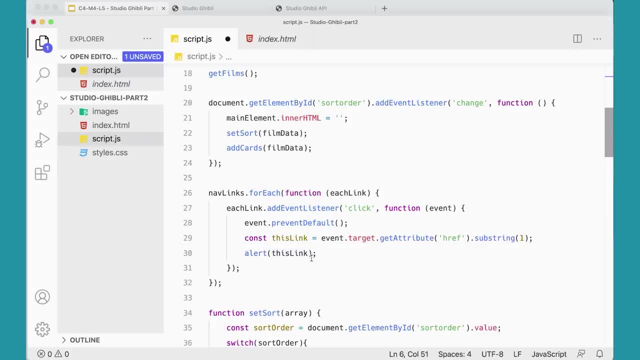 If it's people, it needs to be people. So instead of an alert here, you're going to change this alert so that it's changing those two variables up there. Try to do that on your own and without looking at my answer, because that's a really great sort of micro challenge for you. 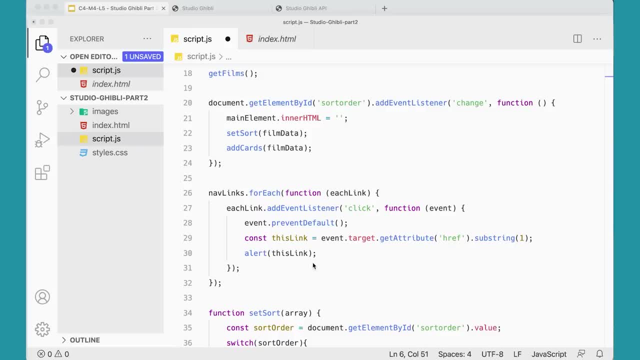 Were you able to do it? I hope so. It should look something like this: The URL is going to be set to this URL plus this link at the end. You could also use the tick marks and do it that way, but this seems to make sense. 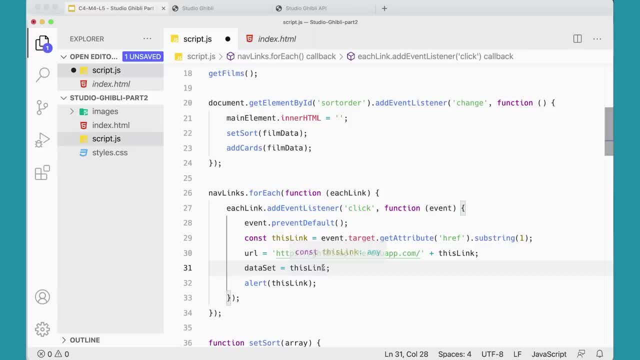 This URL plus this link at the end, and the data set gets set to this link. I don't need this anymore. that can go away. And then I'm going to run a function called get data. I'm going to get data. I'm going to pass in URL. 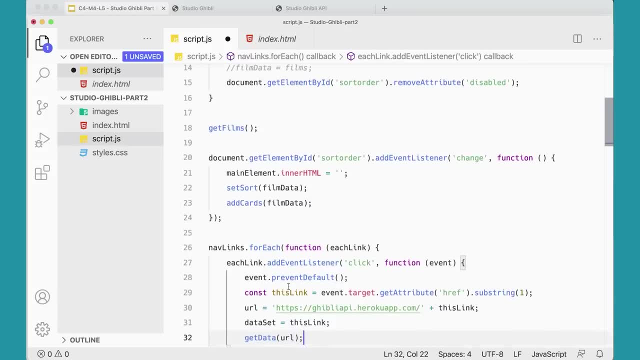 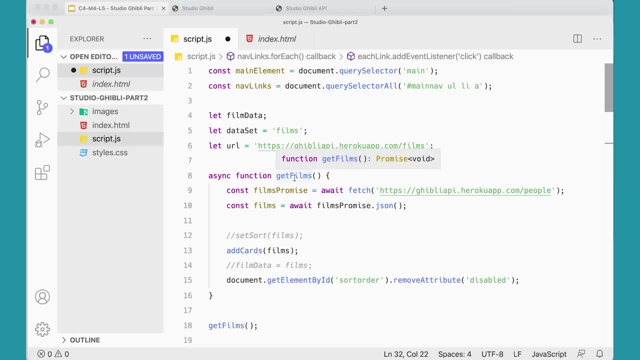 This function, get data- is really going to be the get films function up here. I'm going to Change this to get data, because it's no longer just about getting the films. It's now going to be about getting data, because the data could not be phones. 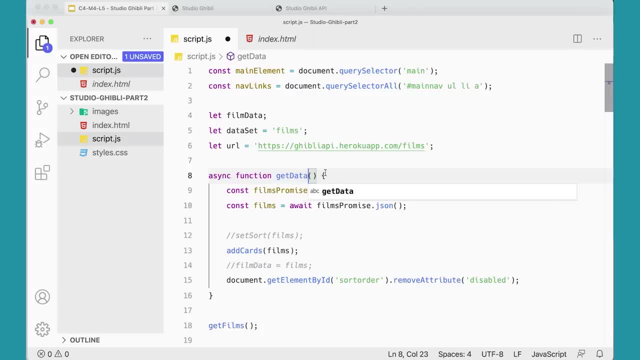 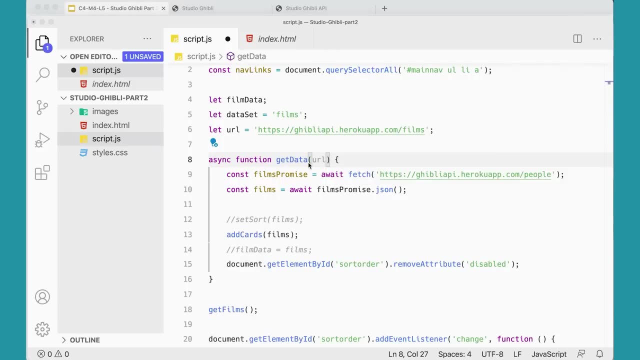 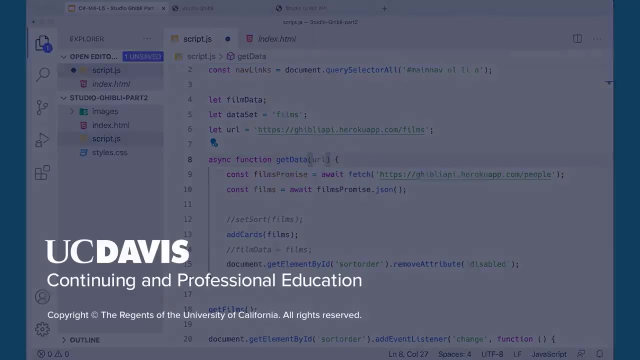 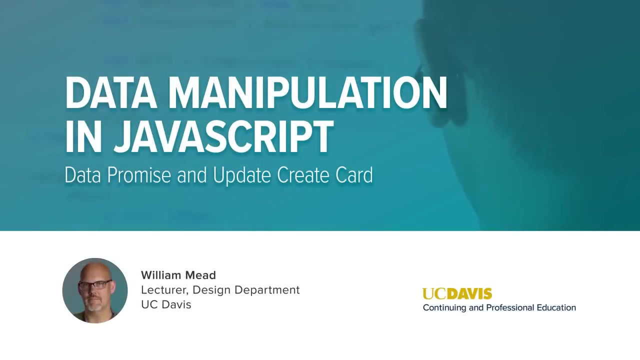 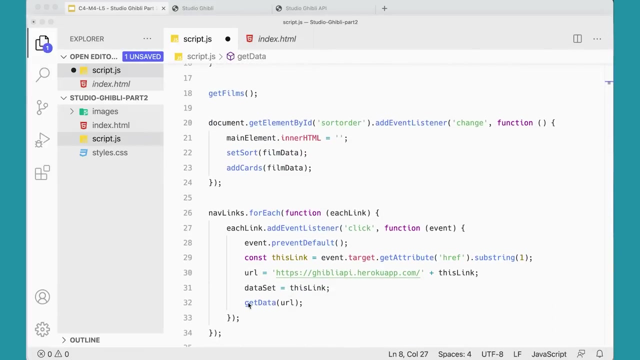 It might be people get data and we're going to pass in a URL. We will finish fixing up the rest of this function in the next video, because otherwise this one will get really long. In the last video we updated our nav links function and we're changing. 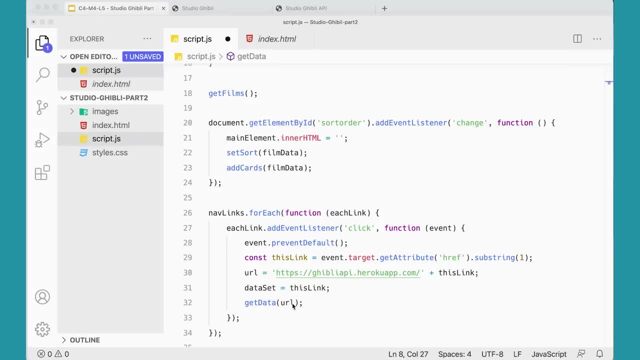 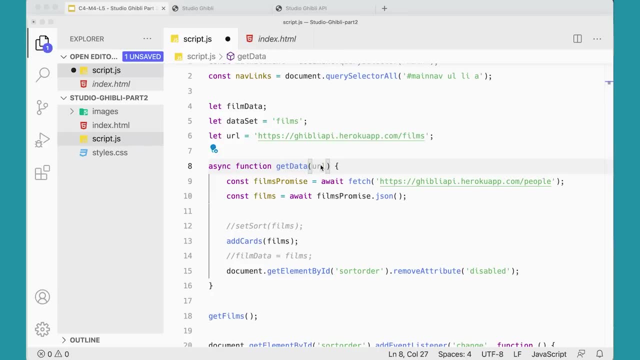 We're running the get data function down here and passing in a URL which is really our get films function, which I've changed to get data up here. We're passing in a URL here, So over here this now becomes not this URL. 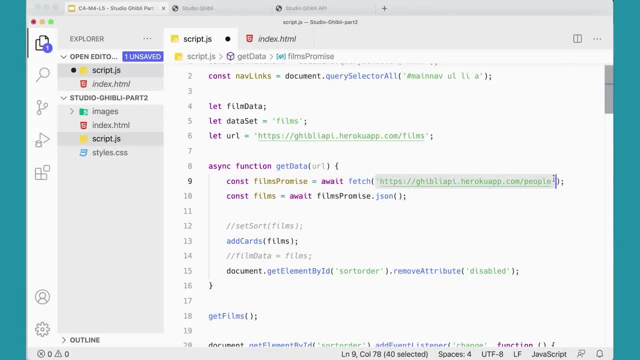 but whatever URL is passed in URL Got the quote there. We're going to fetch the URL and this is no longer really a films promise. We're going to call this a data promise, Data promise. So that means this needs to become data promise as well. 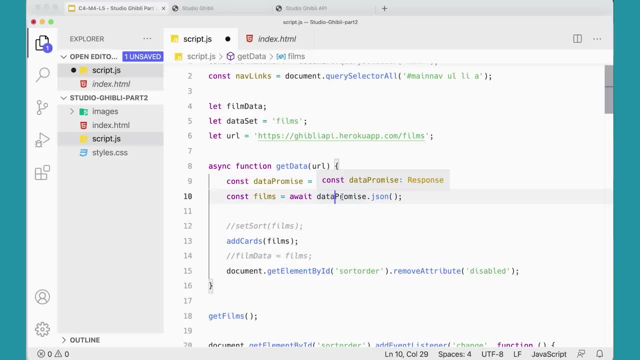 Just kind of changing this a little bit to make sure that it works And over here this is no longer necessarily films, This is now data. Next, we need to do something about this stuff, because set sort is only really going to work if we've got films. 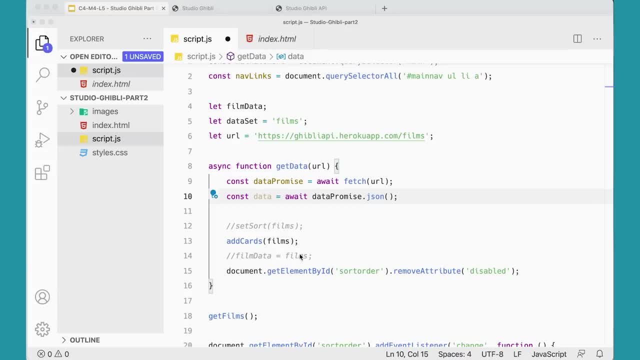 And then the film data is only really going to work if we have films. And then also we only need to remove this attribute disabled if we're on the film page, because we're not going to do that Sorting or any of that other stuff for any of the other pages. 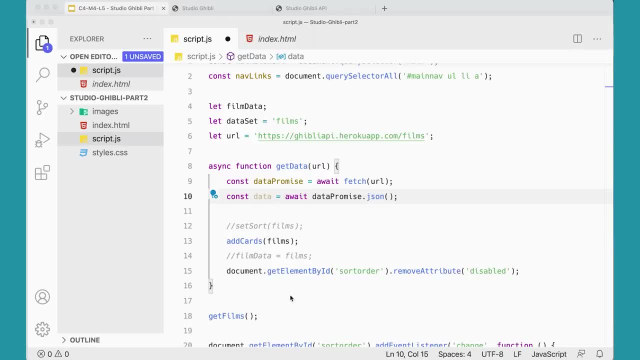 So we need to do something a little bit differently here for this part of this function. So I'm going to take all of this out And instead I'm going to put in something that looks like this: If dataset is the same as films, 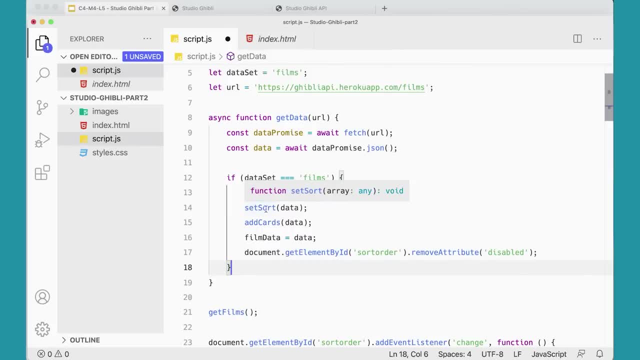 then I'll empty out the inner HTML, set the sort to data, add the cards. I'm passing in data. it's not films anymore, it's now data. The film data is data and I'm removing that disabled thing. Then I'll have an else. 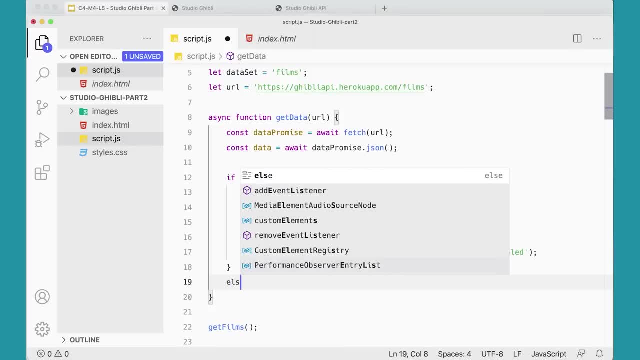 that's going to handle all the other types of cards And really that's just going to have a couple of things in it. It'll have the main HTML. we'll set that to empty, so we'll put that in there and then we'll. 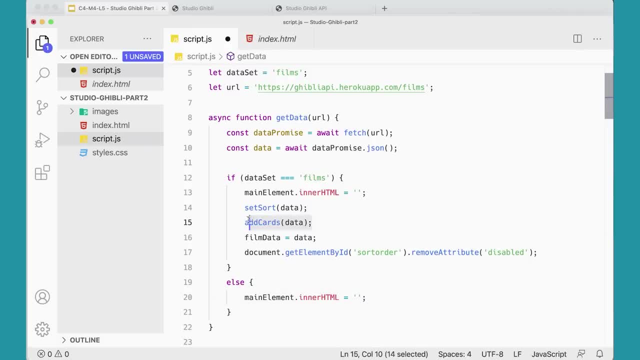 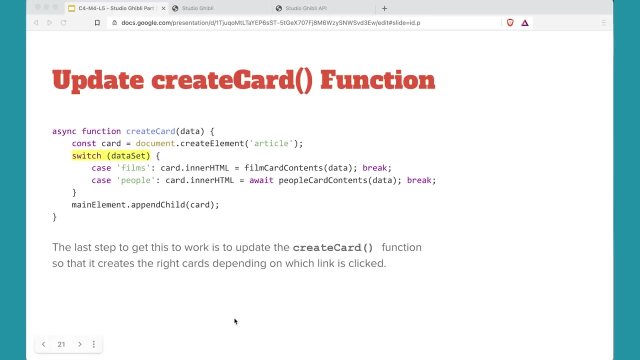 add the cards, We don't need to do anything else. if it's any of the other pages, Save that. The last thing we need to do before we can test this and see if the mess we've made is working so far- and to check on this is we need to update this create card function to handle. 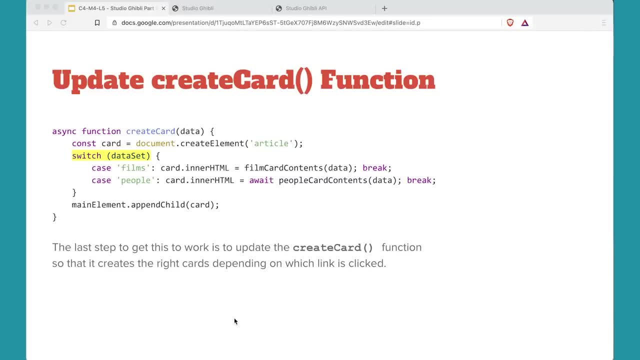 adding the right type of cards depending on which link is clicked. So we've got our function: create card, we're passing it- some data and then, based on the data set- remember we created that variable which is either going to be films: 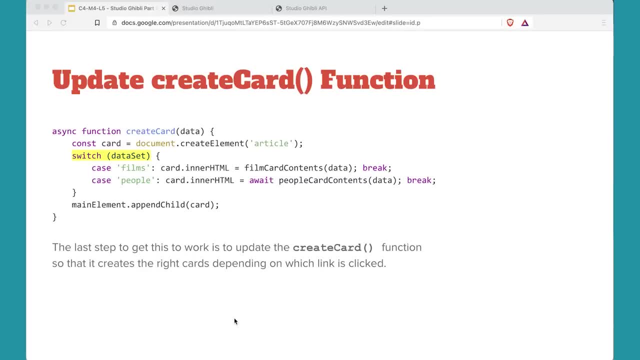 or people or vehicles or whatever it is. We can use a, we can use that in the switch statement to swap in the correct thing based on. based on that case, And if it's films, we're going to run the film, we're going to add the film card content, so we'll run the guts of the card that way. 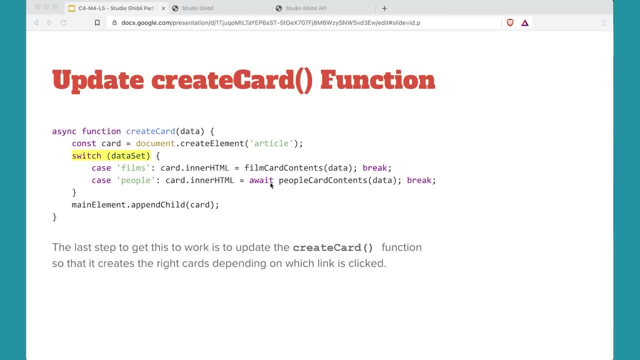 If it's people, we're going to do the await, because that has the asynchronous functions in it and do that one there. So let's go ahead and add this to our create card function. update our create card function. Currently, right now, we only have 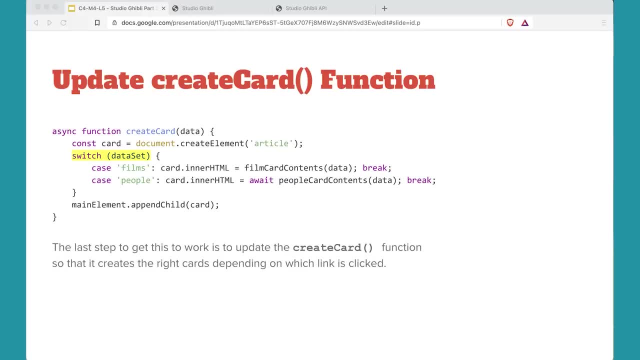 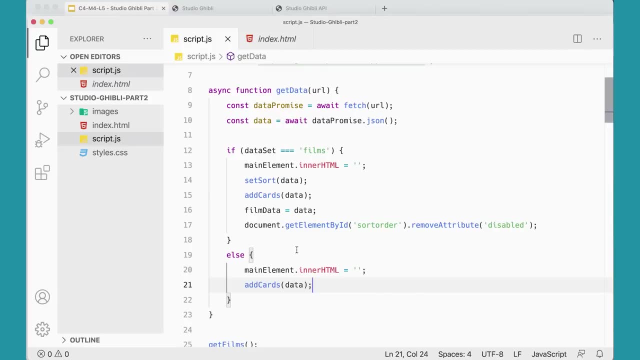 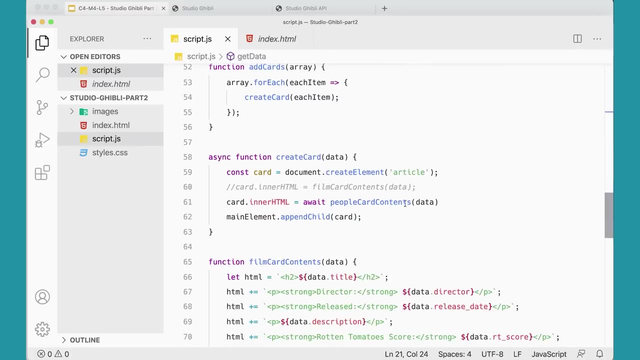 cards for films and for people. so we're going to have to add the other ones later, but let's see if at least this much works. So, coming in here, I'm going to come down to my create cards function Here. it is here and I'm going to get rid of these two things. 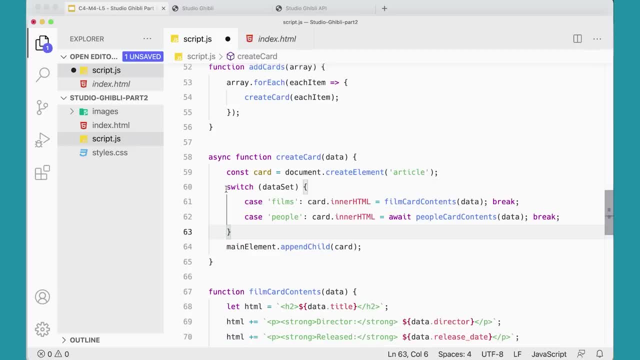 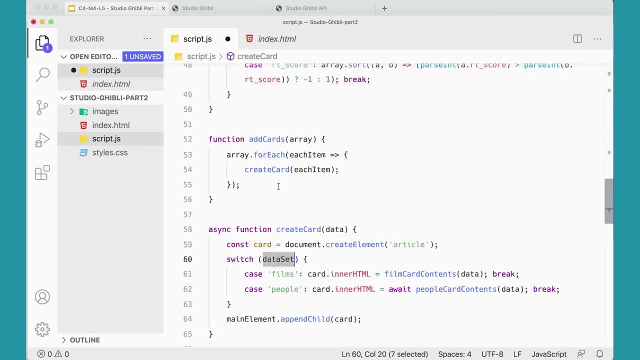 And put in the switch statement instead. You're going to have to type it. I pasted it in, but you're going to have to type it. Switch data set: This is a variable that's currently global up here. data set: Currently set to films by default. 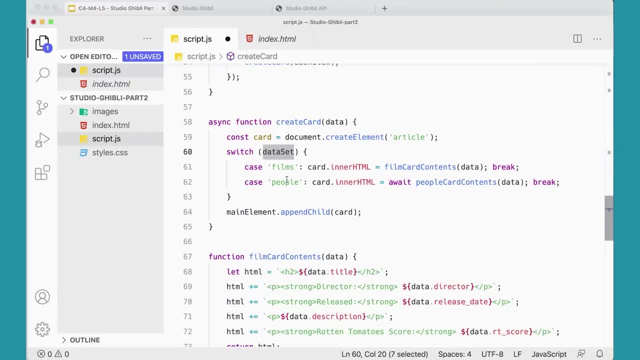 So based. it's either going to be films or people. right now I mean it could be the other ones, but- and that would be bad because those won't work- But we're going to set our inner card content. We'll use the film card contents if we clicked on films, and we'll use the people card. 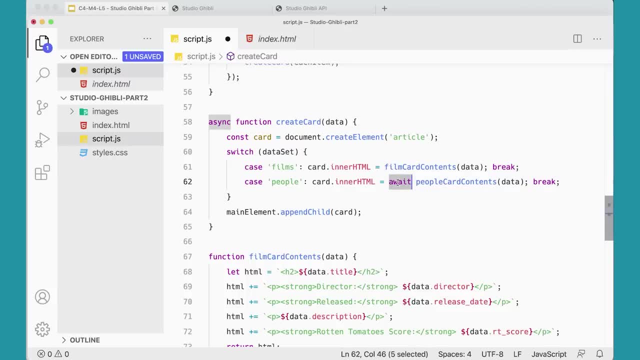 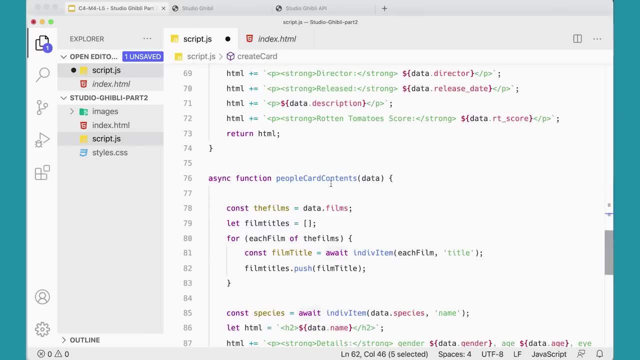 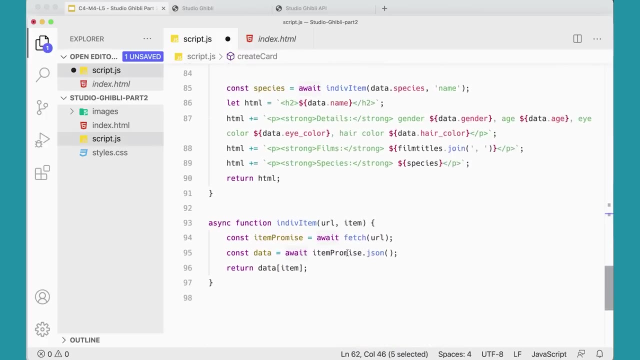 contacts if we clicked on people. And again we have to have the await here and that's why this function is set to async, because down here in people on the people cards, we are actually doing some additional asynchronous functions here to get the people. 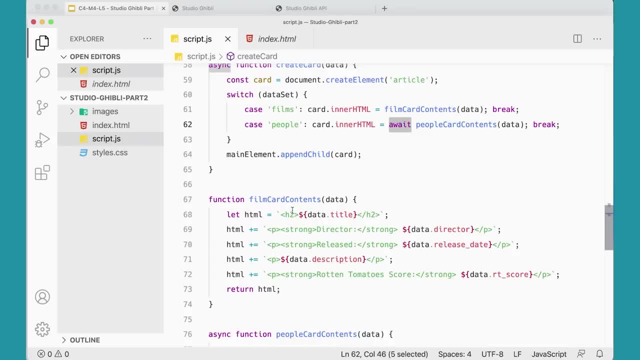 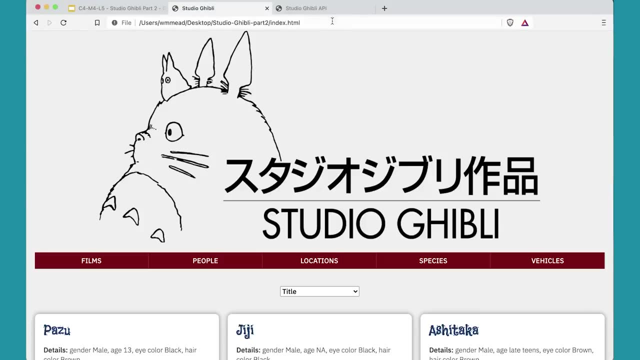 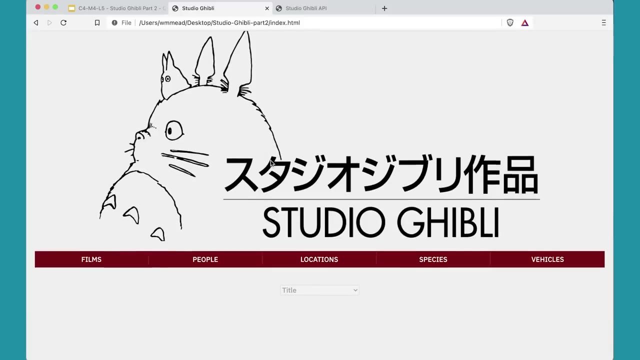 All right, cool, With all that in place, we'll see if this actually works. Hopefully it does, and I didn't screw anything up. Let's see over here I'm going to refresh my page. Come up here, click the page and something has gone wrong. 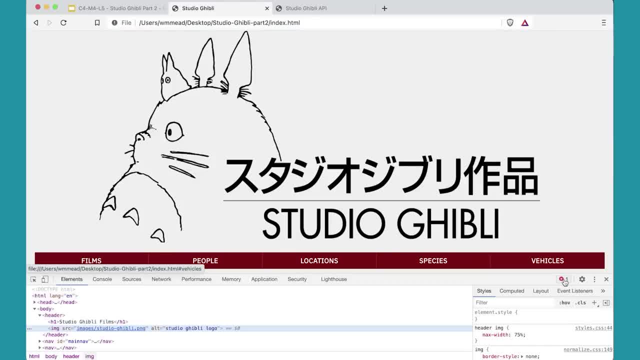 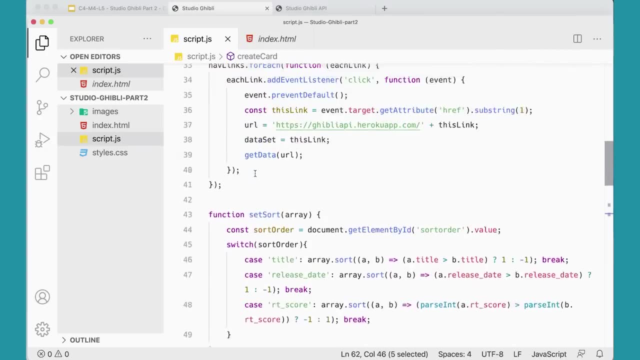 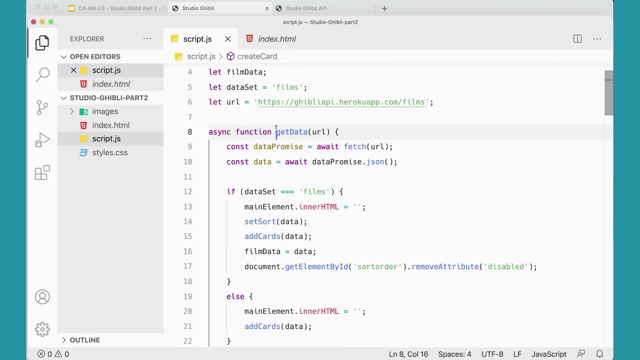 Inspect. I have an error here. Let's go see what that error is. Reference error: Get films is not defined on line 25.. I forgot to change something because I'm no longer using get films on line 25.. Oh, get films. That needs to be get data with the URL. 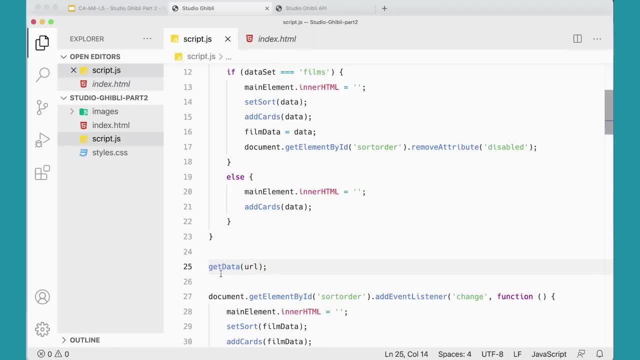 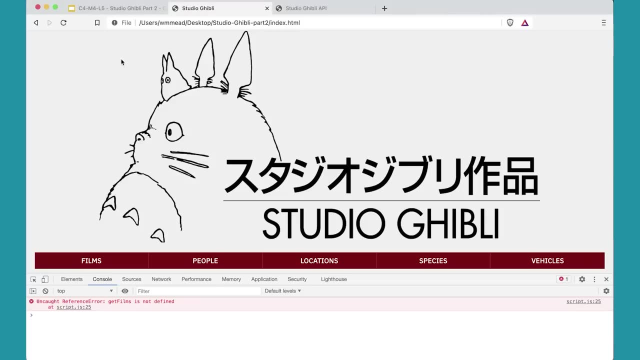 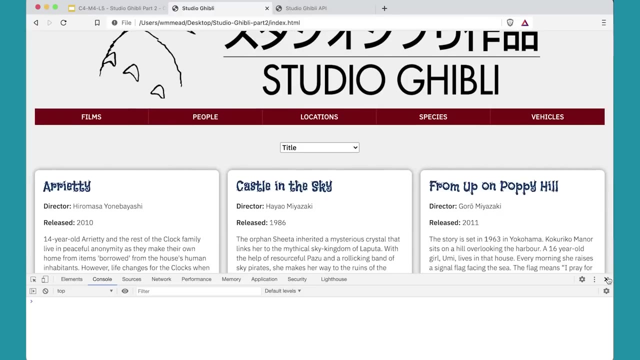 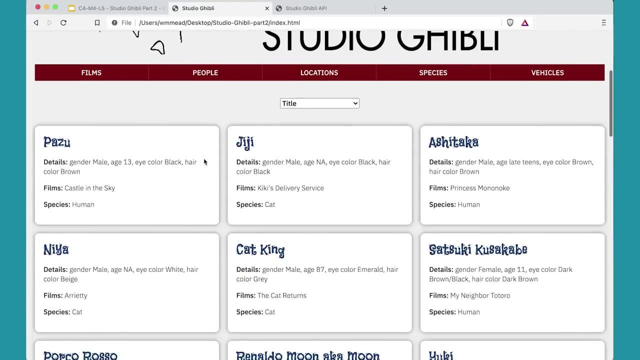 Get data Passing in the URL and again the URL by default is the one with films, so that should get us films. Let's try it again And look at that. I have films. If I click on people, I have people. 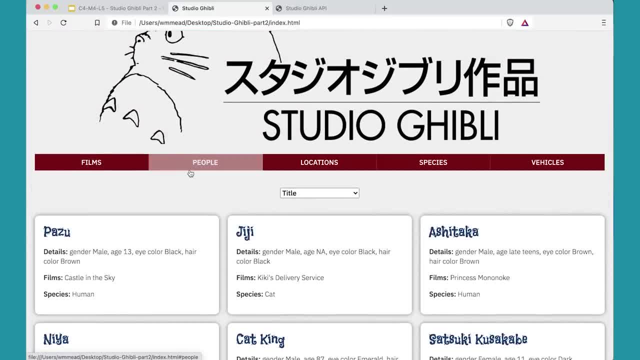 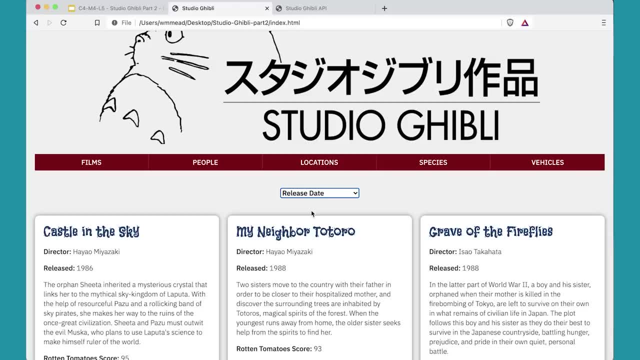 These other ones won't work yet. Don't click on those. If I'm on films, then this title thing will work. I'm going to have to do something. I'm going to have to do something to hide this if I'm on the other pages, because it's not going to. 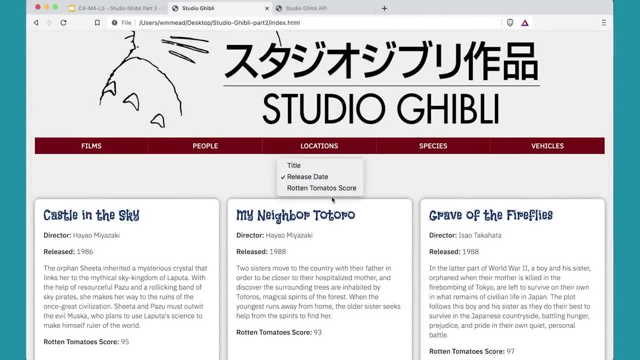 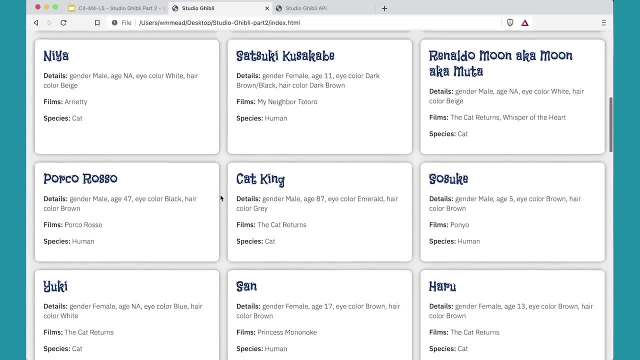 work for the other pages. We'll get to that. That's working fine and it's nice and fast because it's actually loading the data that was loaded once. You'll notice that when you go to people it takes a second to go get that data. Cool, That's working so far. That's great. 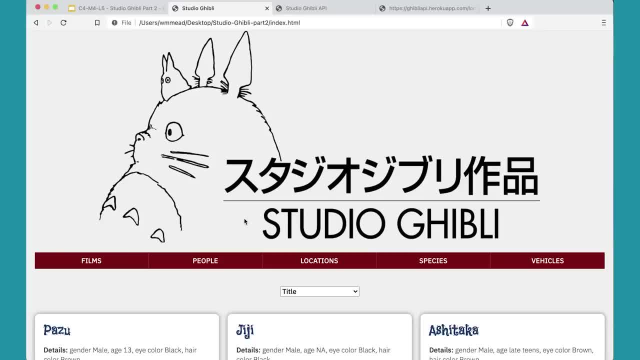 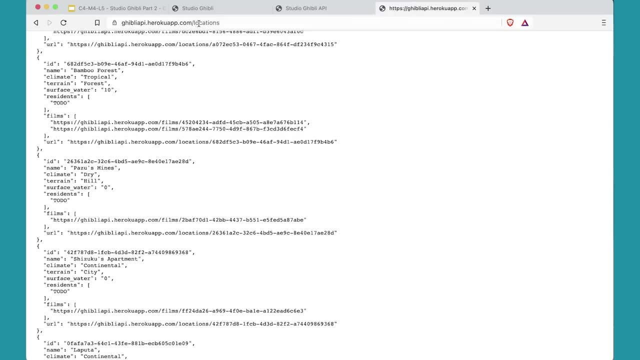 We have so far gotten the films and the people to work, and that's great. So now we're on to locations. But if you go look at the locations endpoint, which is this URL: slash locations instead of people or films, it's just slash locations at the end. you'll notice that in the data in places, 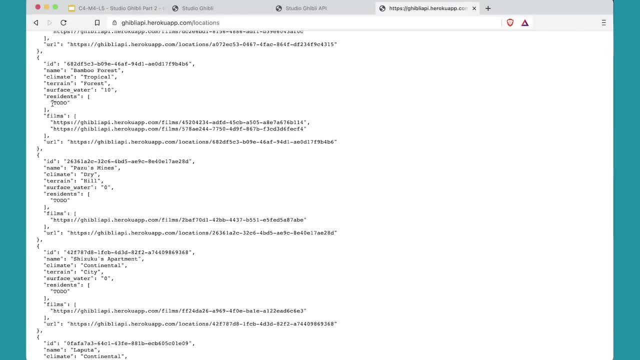 instead of having key value pairs here, it just says to do Okay To do, To do under residence. So whoever created this data never got around to finishing these pieces And because these things are not actually correctly marked up, I mean it just says to do: 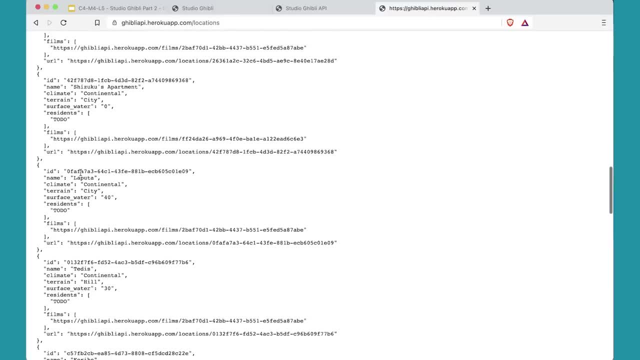 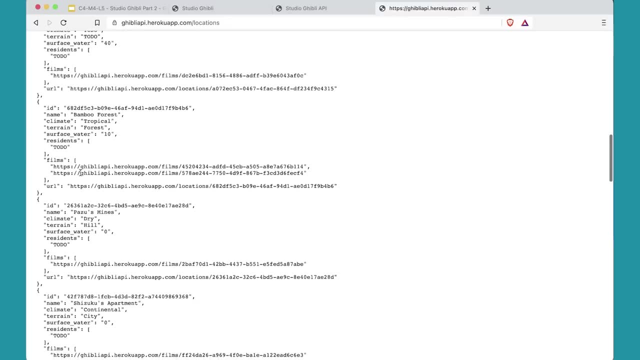 in here. it's going to cause errors, It's going to cause problems. So, because of that, that's a good thing, But we need to do a few different things. We need to do some error catching. So this is actually a really great thing that it's not finished, because it helps. 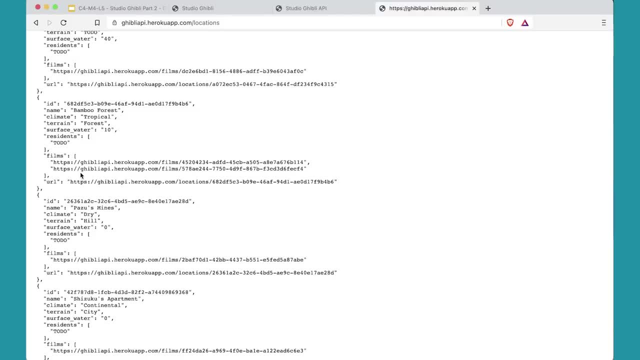 us learn something new in the process of doing this next part of this project, which is going to be kind of fun and interesting and important to know. It's possible that when you use a third party API, you won't always have access to it, or some things won't work, or things and some things. 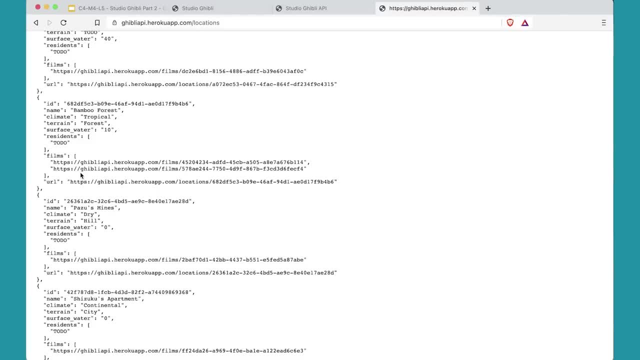 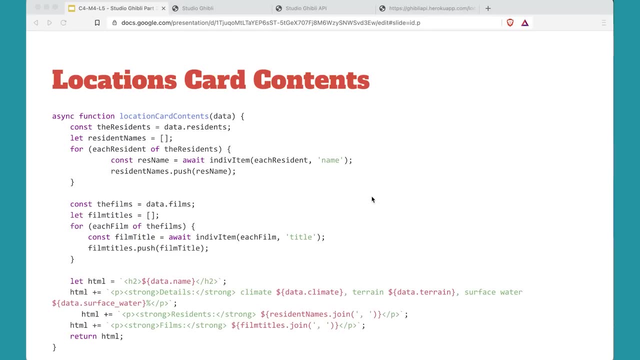 haven't been entered properly by somebody else And that you're going to get an error. So we want to those errors and do something with them. Here is the function for the location card contents as it is currently, and you're gonna have to pause the video and type this in, and really it's probably. 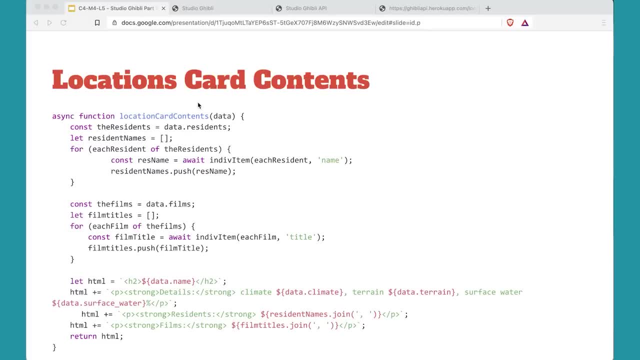 best to take the people one copy and paste it and then make minor changes to it, then type this all from scratch. but you could type it in from scratch. it's not that big a deal. it looks long, but you'll notice that these parts are really very similar. so this, this part here, is very much the same as that. so 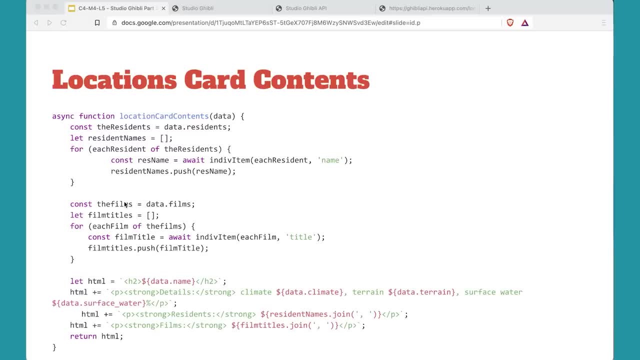 you could use even copy and paste within these to get them to go and then down here and making my HTML variable and filling it with the data that I get from my card. now this is gonna cause I'm gonna get some errors in here because it will get past to do instead of a URL for some records and that's not gonna work. 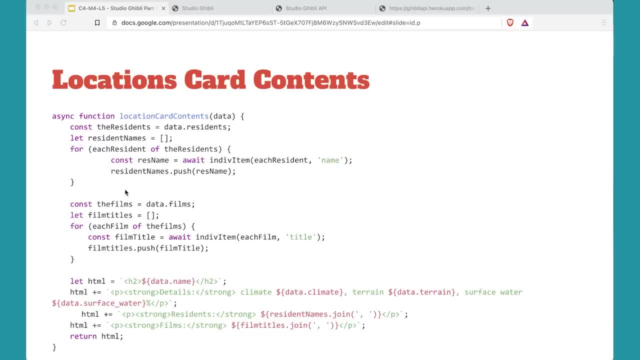 so we're gonna get some errors here because it will get past to do instead of a URL for some records and that's not gonna work. so we're going to have to fix that in some places. but this is a good place to start, so i'm going to go over. 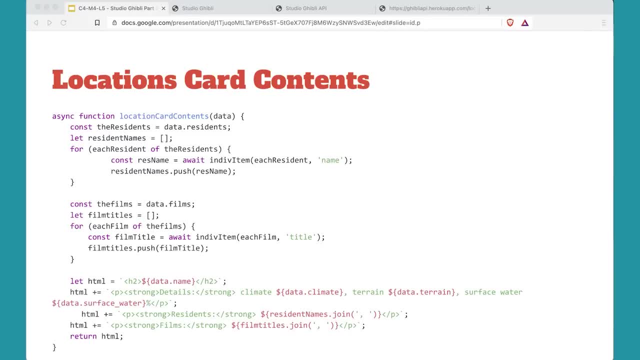 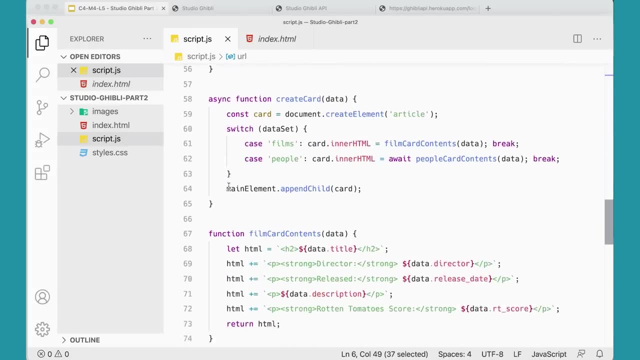 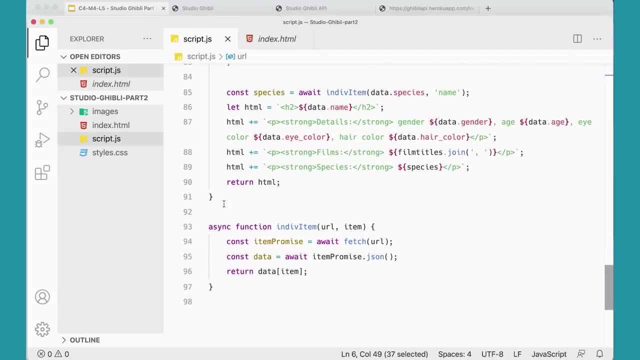 and add this to my uh script file here and come down to close to the bottom here. i've got my people card content here and i've got my async individual item there. i'm going to leave that at the bottom because that's a helper function. i'm just going to add this one. 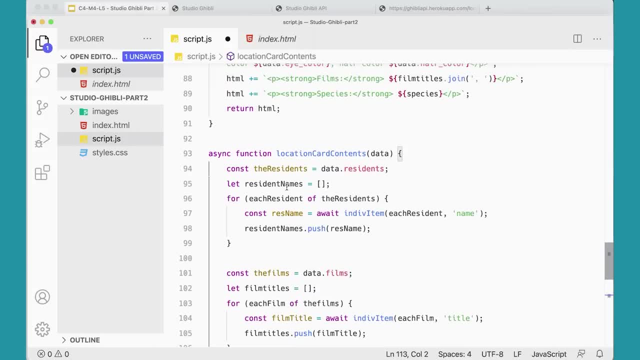 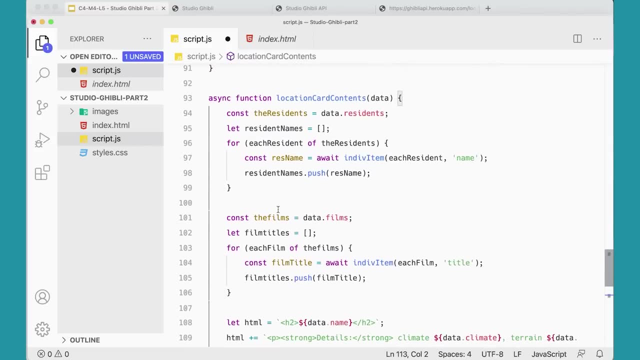 in here. you're going to have to type it in, but i've copied and pasted it to cheat. i've already typed it many times before, so i didn't type it again and have you watch me type it. but go ahead and add this in here. this is the whole thing. 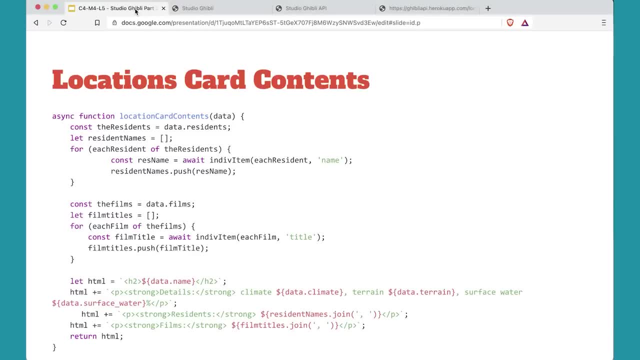 and again, i'll go back to the slide here so you can see it and pause this, so you can get this in there and make sure that it's right, pause this and come back and when you've gotten this script, when you've gotten this function on here. i realize that it's long and i do apologize for. 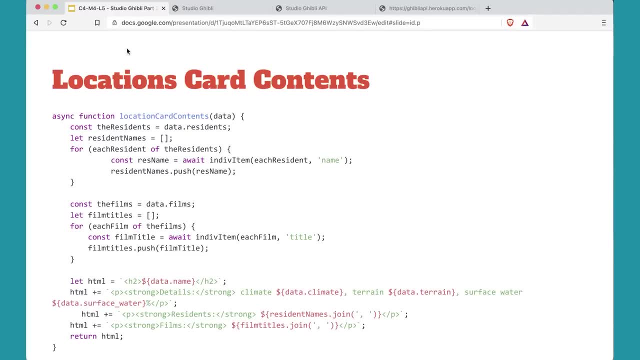 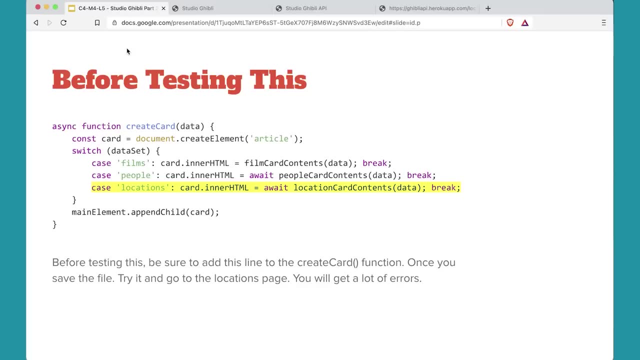 that all right, great. so now that you've gotten this in here, before you test it, we need to make sure we add the locations case to the create card function so that it will actually go and create those cards and get that content in there. so let's do that next. that's really pretty easy. 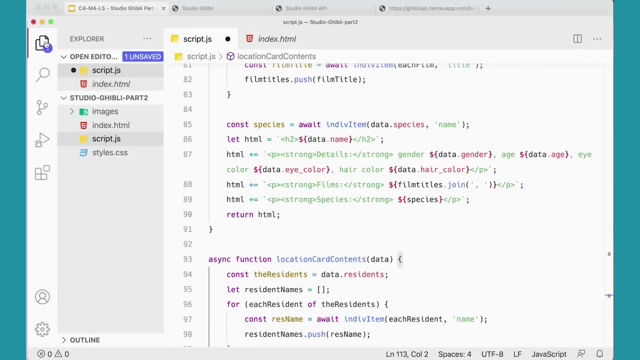 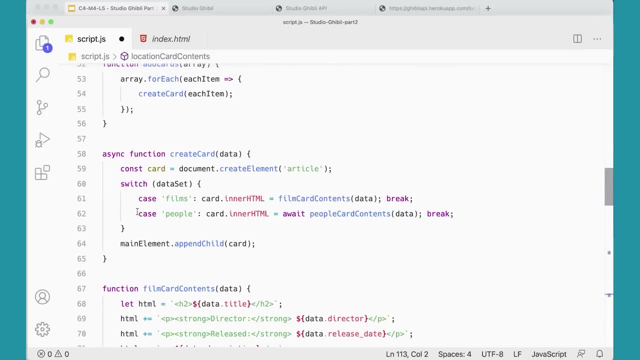 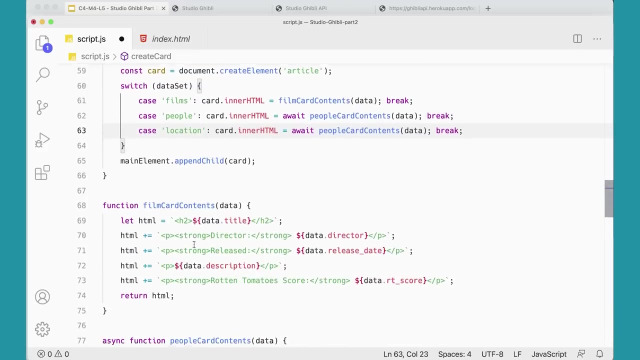 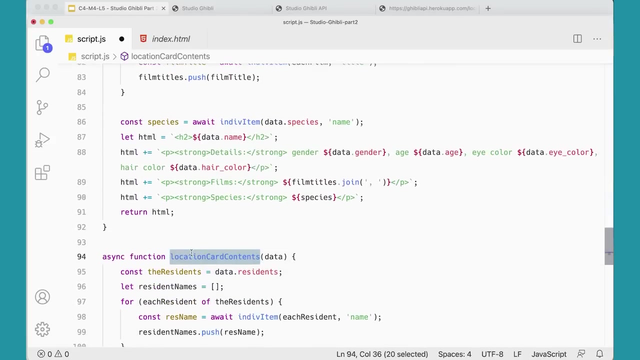 if we come back over here to our- i'm going to close my explorer here- to our create card, then you're just going to copy one of these, that one, change this to location and then i need to get the this name. i'm going to copy and paste. 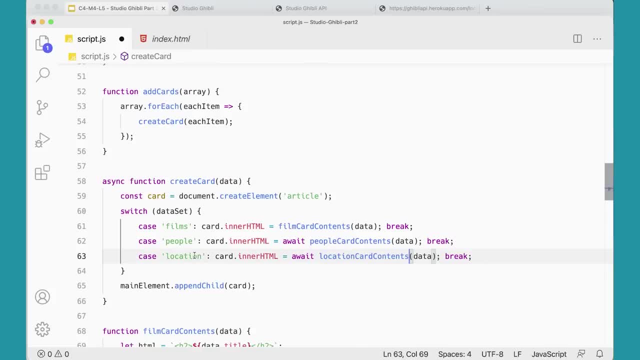 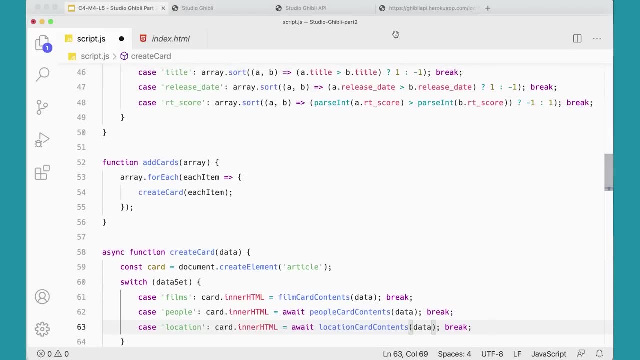 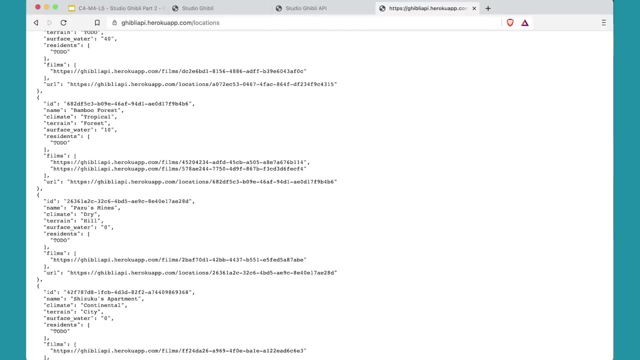 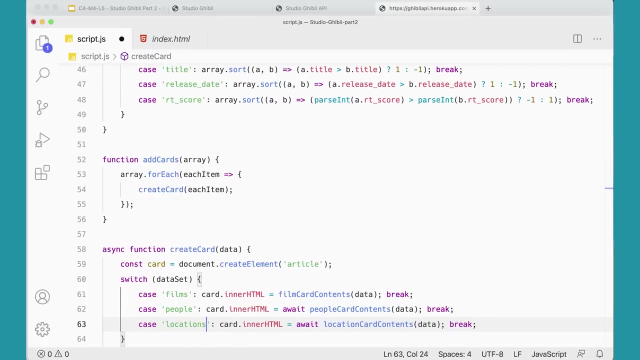 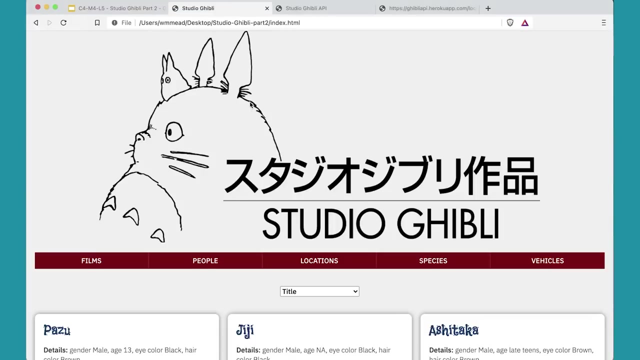 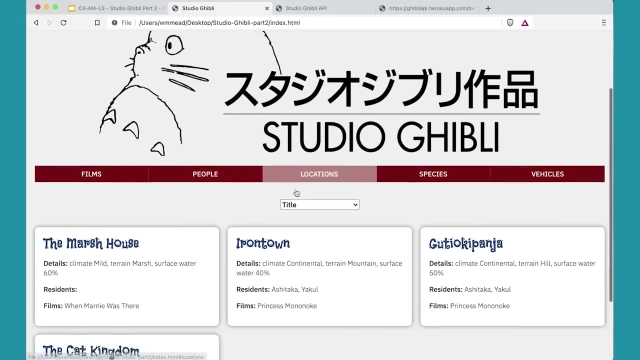 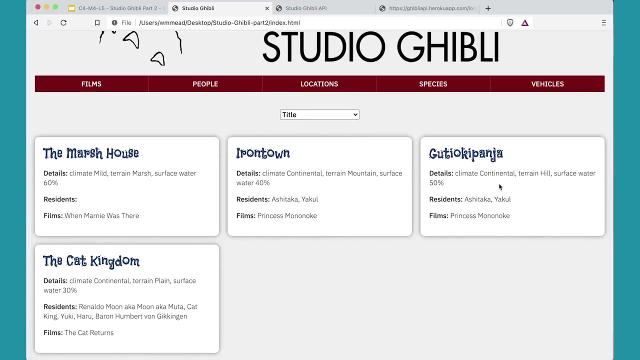 paste it there now. is it location or is it locations? well, let's find out here. data set over here. it's locations. it's always good to check on these things. okay tod watering and okay locations. great, let's save it and i'm going to come back to my webpage. 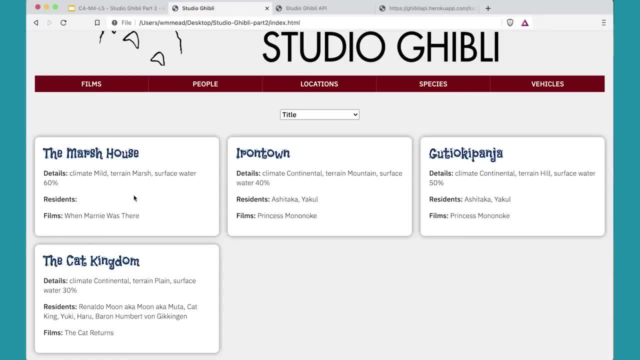 refresh and when i click on locations you'll notice it's coming in, but i've only got four cards that actually have residents listed and this to be This one is just an empty array. And if I were to inspect and look over here in my 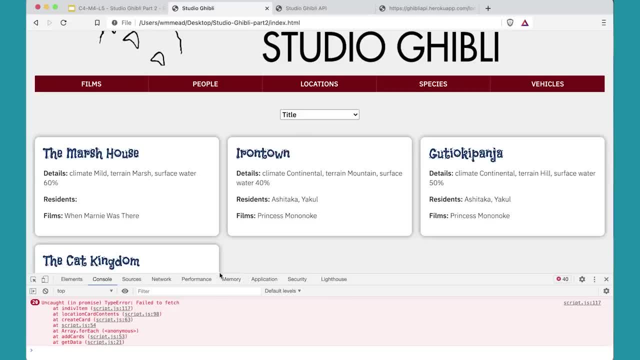 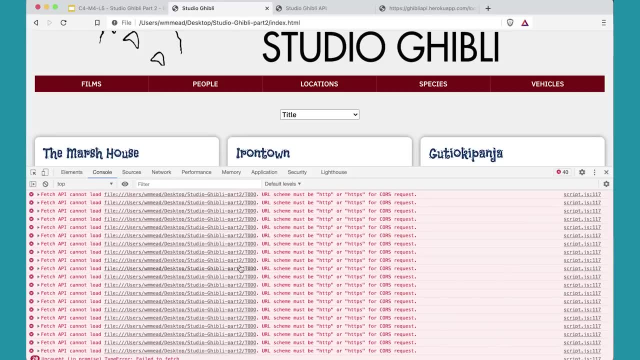 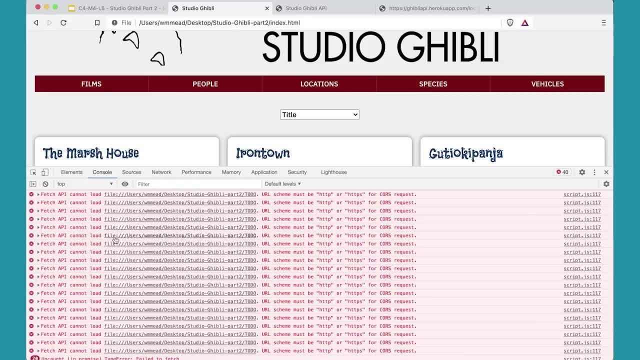 It doesn't know what to do is here. It's looking for an API. It's looking for a URL that's slash. to do That doesn't make any sense, So that's causing an error. So we'll look at how we can fix that in the next video. 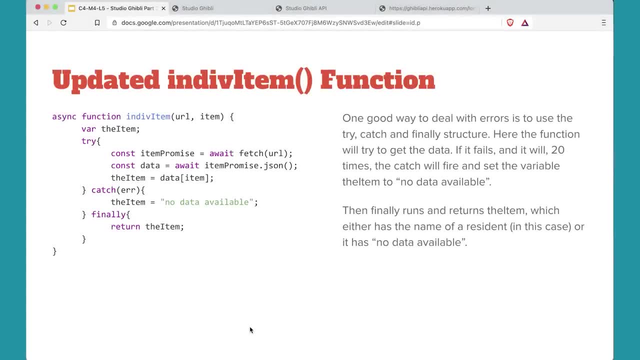 One thing we can use to try to catch some errors is the try, catch and finally structure. that will help us try something And if it doesn't work or if we catch an error, we'll do something else And then finally, we're going to return something. 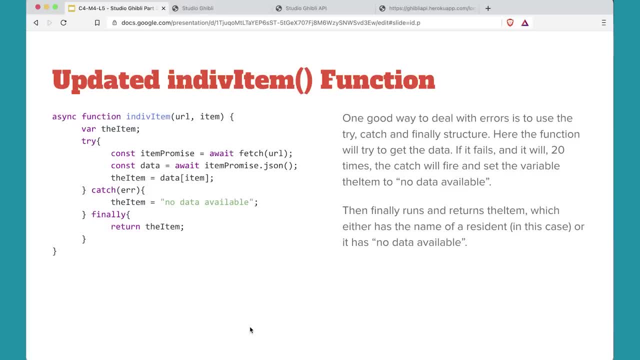 And in this case we are going to get a lot of errors. So I'm going to update my helper function for getting an individual item with this try, catch and finally clause to see what happens when this runs here. So let's go ahead and add this to our script. 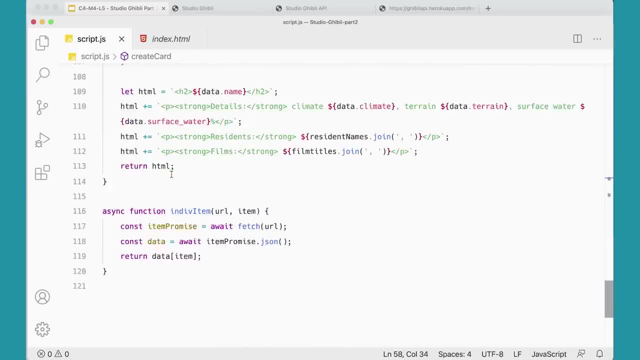 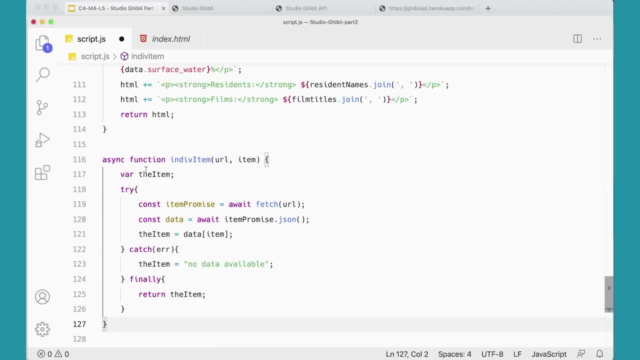 Down here at the bottom. I have my helper function here And I'm just going to replace this one with the version that has the try catch. So I've got the item. I'm getting the item here. Try the item equals data item. 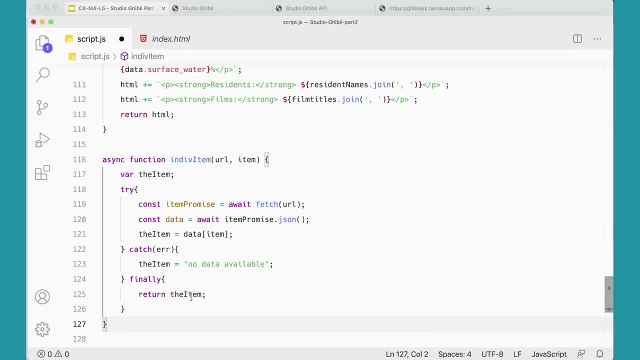 Catch the item. no data available. Finally, return the item. So the item is going to get returned one way or another. It's either going to be the data that I want or it's going to be no data available if there was some sort of error. 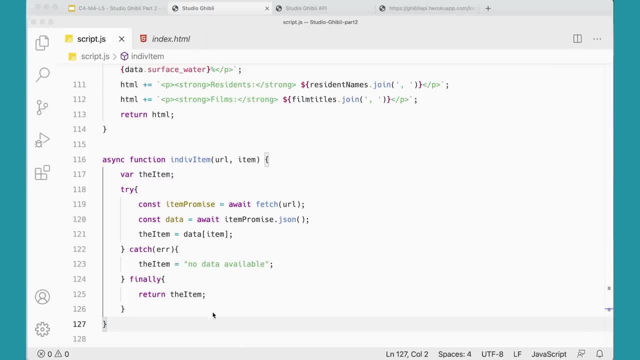 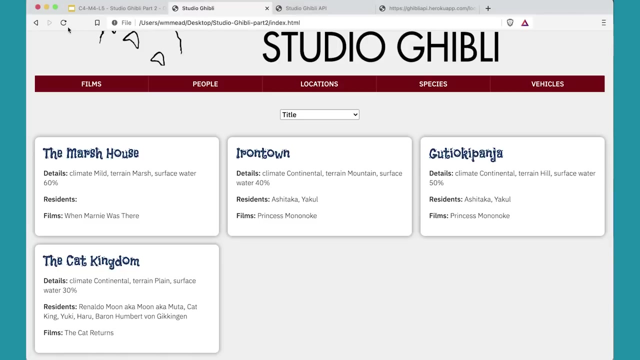 So we've got that in place. Let's give it a try. You're going to have to stop and type this function in or update the function so that it has this, But let's give it a try. I'm going to come over here and refresh. 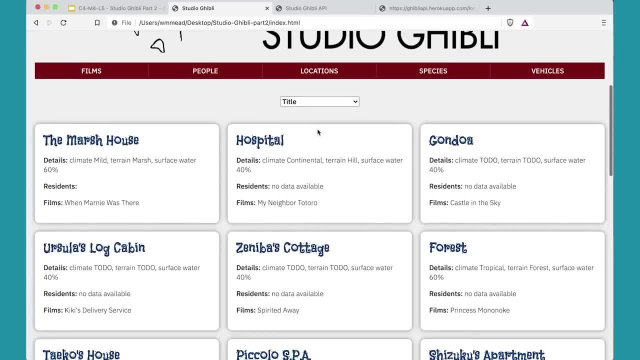 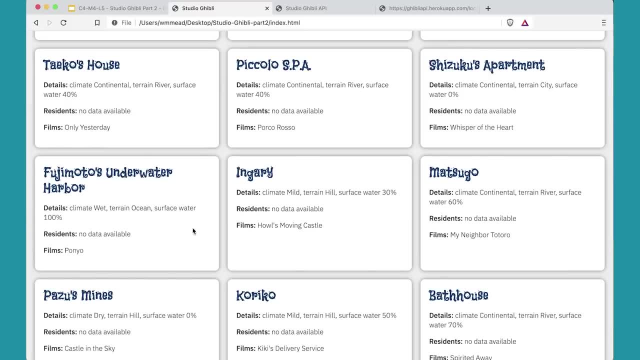 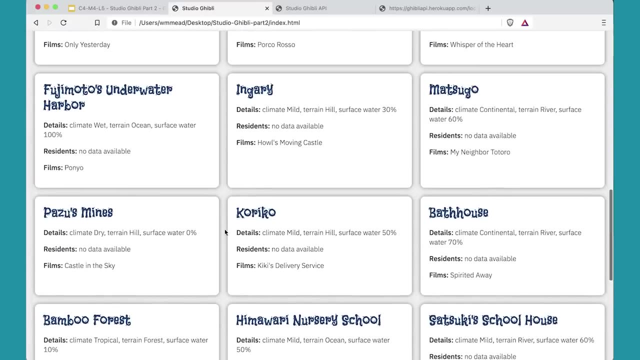 Come down here, click on locations And now you can see I'm getting my locations. It still says no data available here. It says no data available for most of these, but at least I'm getting all of my cards. I may still be getting some errors. 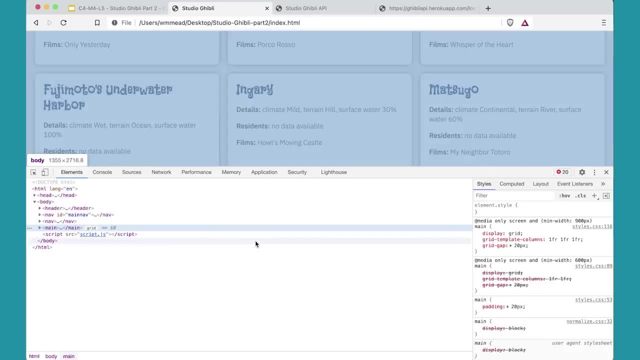 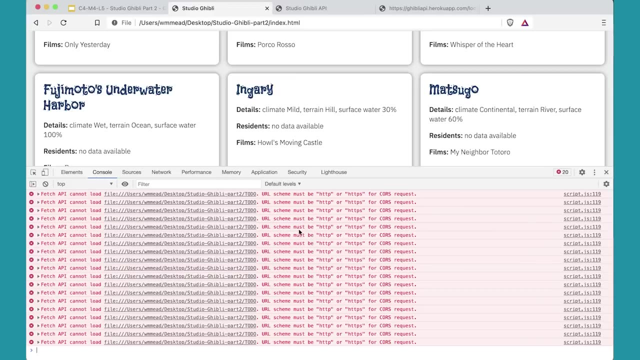 Let's see And look at that. I still have 20 errors over here. It still doesn't like these to-dos. It's still trying to do this, But at least when it's trying to do it and it's failing. 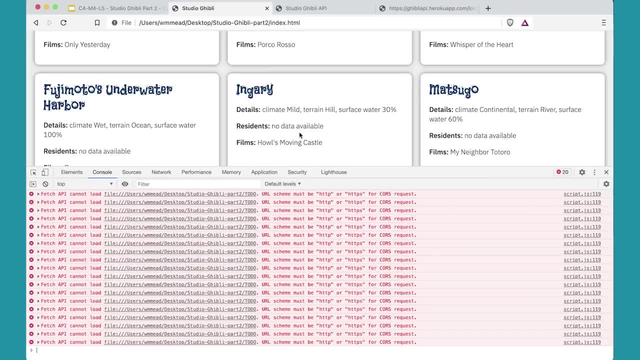 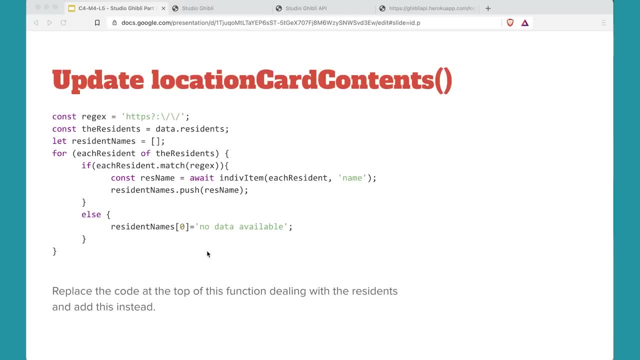 it's then at least putting no data available and not holding up getting my cards. But I think we can make it better still. I'm going to update the code at the top of my function for generating the locations data with this little piece here. 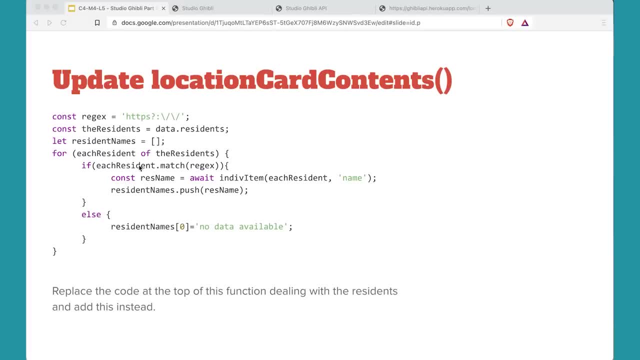 And I'm using a regular expression to check to see if, when I get this, if I'm getting something that matches the regular expression, and if it doesn't, I'm going to set that to no data available and that should help. So let's see if we can get this to work here. 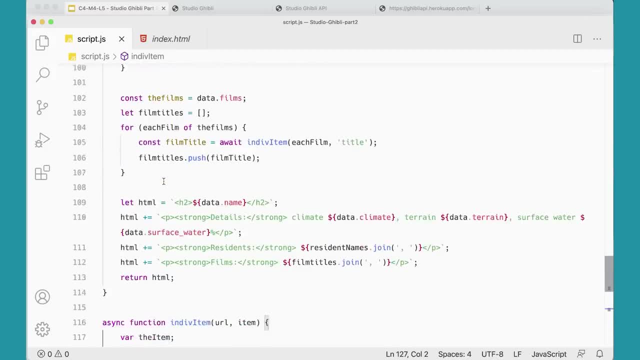 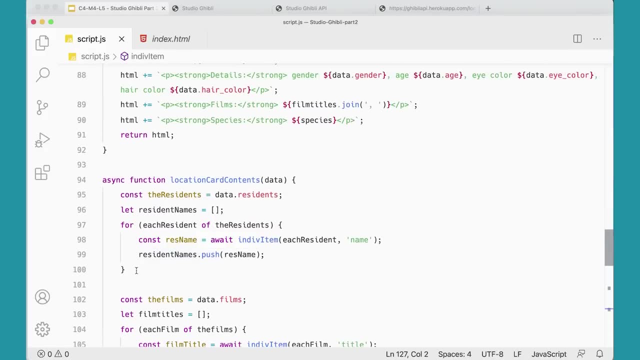 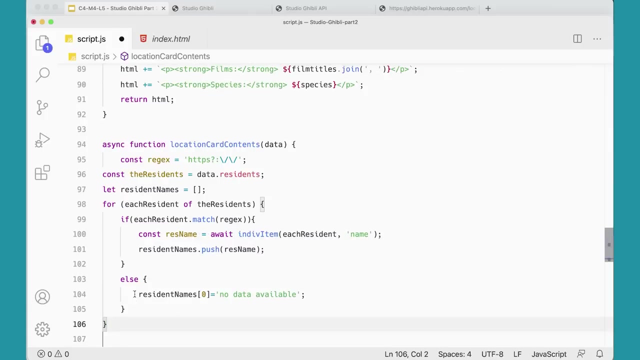 I'm going to come down to this function here Here. it is here for this residence one. I'm going to get rid of the top of this And just replace it with that. I'm going to have that in The residence data. residence. 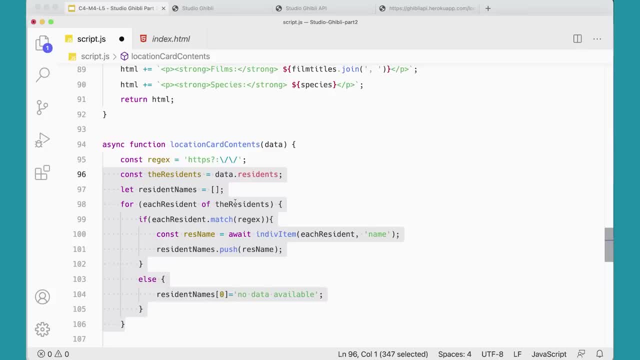 the resident names. I've got an empty array for each resident of the residence. if residents match regex, So I'm going to go through each one of them, and if there's only one, then that's easier. I'll just do it once. 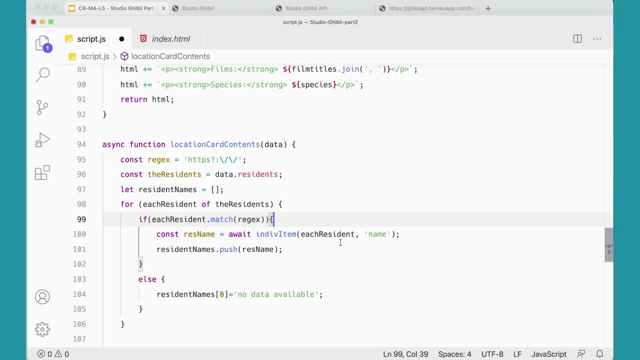 and get the name And if it's- if it matches- I'm going to get the name and put it into the list. If it doesn't, I'm going to set resident name zero to no data available. So let's see what happens when I run this one. 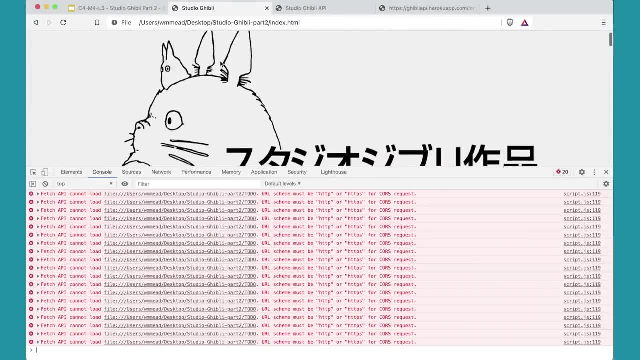 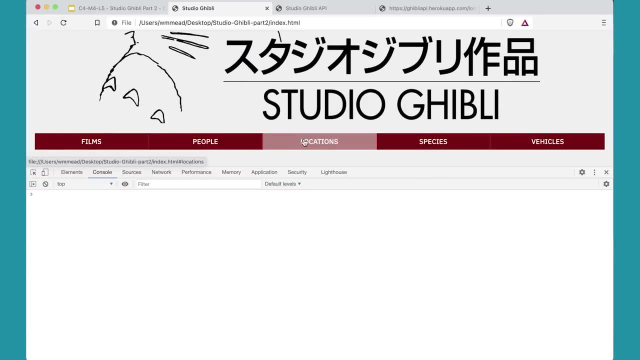 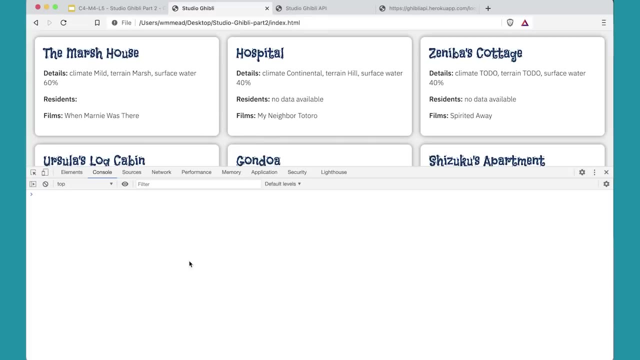 Here I am on my page. I'm going to go up to the top and just click refresh, And now, when I click on locations, I'm getting all of my locations and I'm not getting any errors in my console. Isn't that nice? 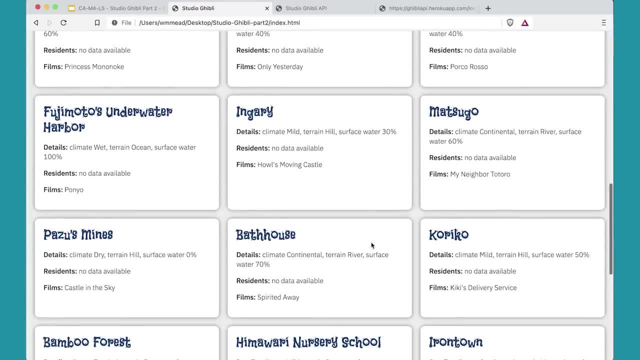 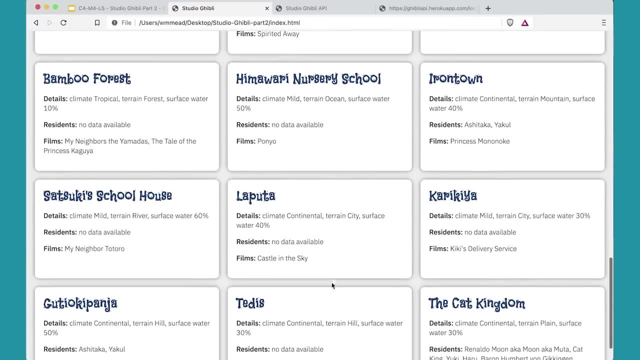 So finally we've gotten this fixed And residence is no data available, and that's fine for the ones that don't have any data. At least we're not getting any errors. So you have to really go through and make sure you can solve for any errors. 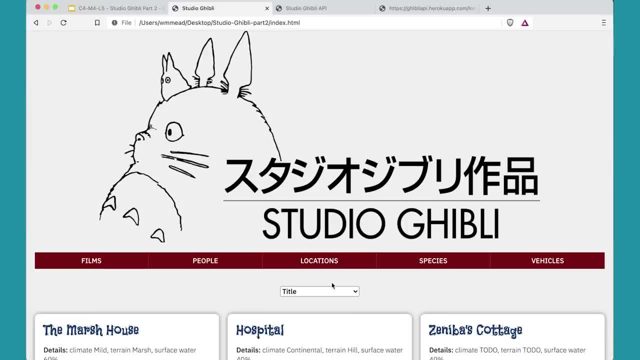 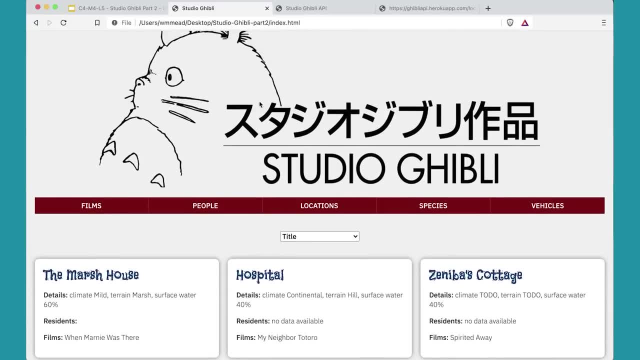 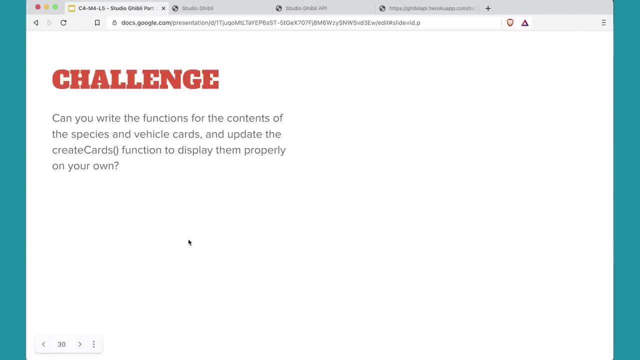 that you might get from your data And make sure that you're not trying to get something that doesn't exist and handle it properly. Okay, great. So now the next challenge: can you write the functions for the contents, for the species and the vehicles cards? 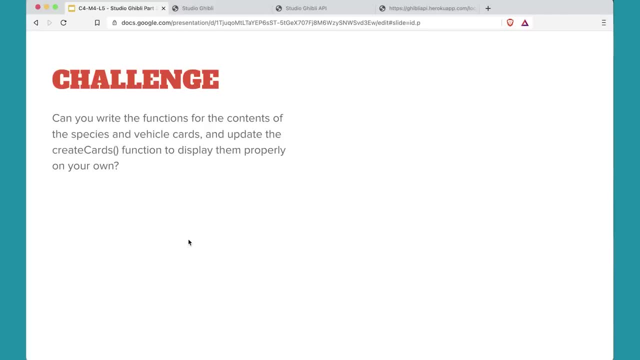 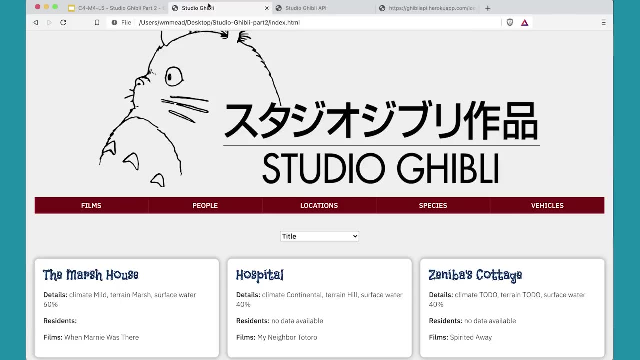 and update the create cards function to display them properly on your own. Try to do it. The last two pieces. for these last two bits we've done. films, people and locations meet species and vehicles. The last two pieces aren't that difficult. 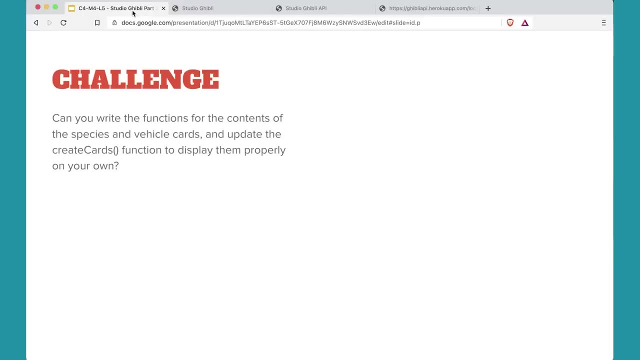 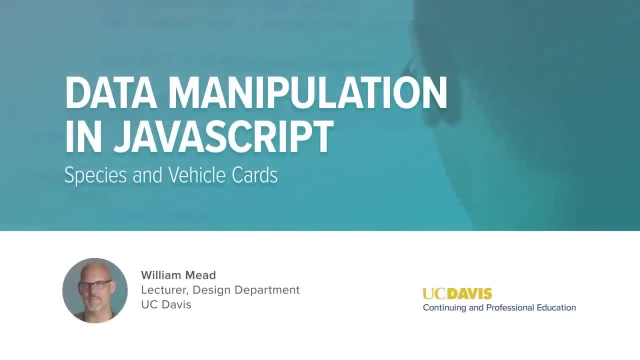 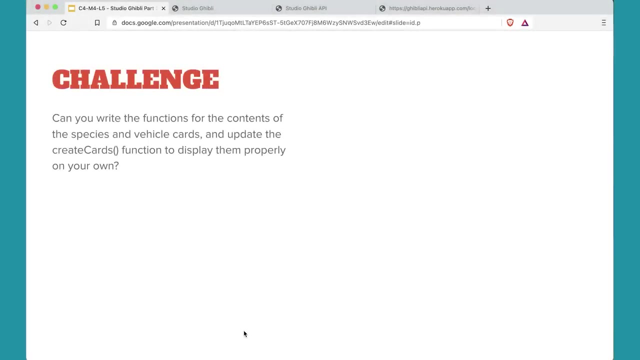 They're not that different from what we've done, So they shouldn't be too hard. See if you can do it on your own. Were you able to get the challenge to work? Were you able to write those functions for the species and the vehicles pages? 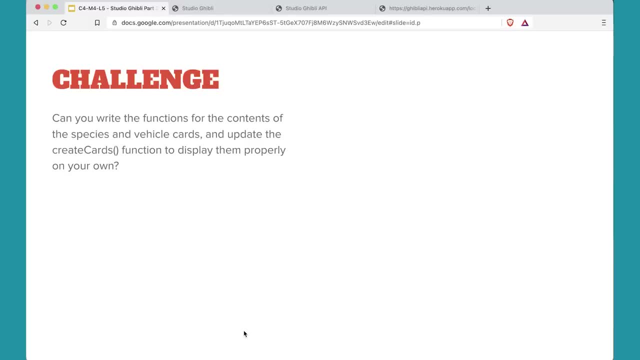 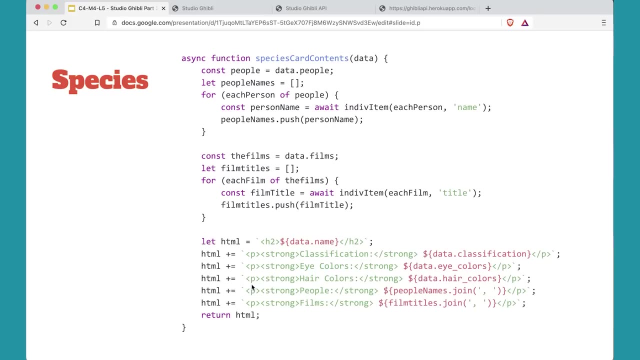 and cards, or did you get stuck? Hopefully you were able to do it. The species one should look like this. It's not too surprising. It's very similar to what we've done. Hopefully you came up with the same thing or something similar, and I'm generating the HTML and returning it here. 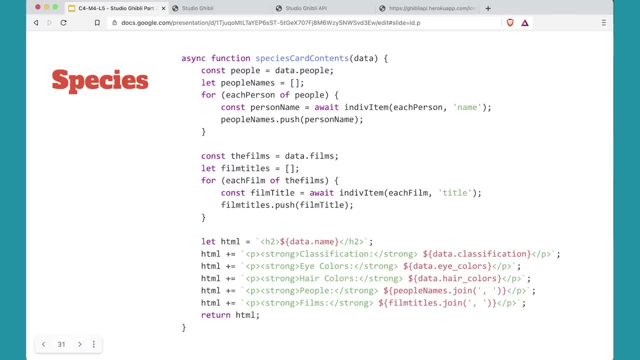 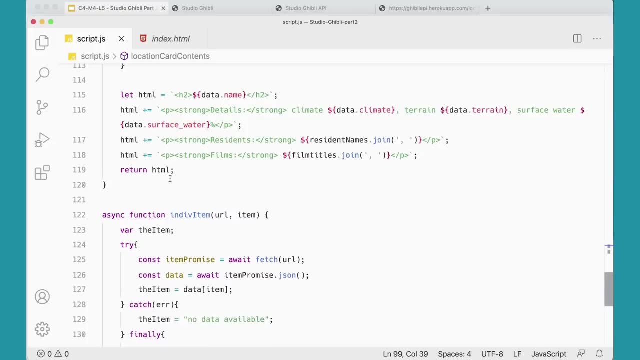 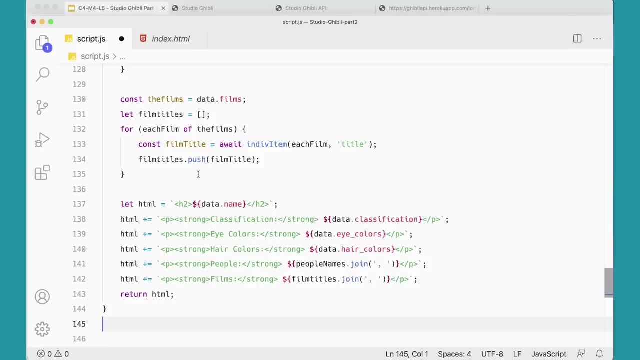 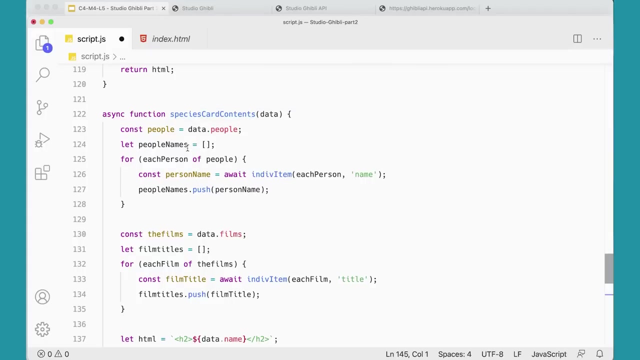 So that's all fine. So let's go ahead. I'm going to go ahead and add this one into my script over here, and I already have it copied. I just need to paste it and I'm going to paste it here. So we've got species card contents, people, people names, all that kind of stuff. We're going. 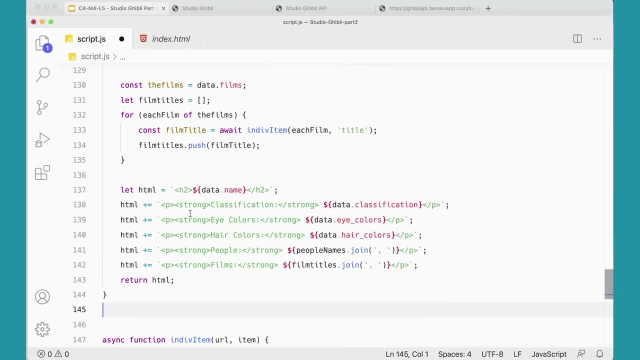 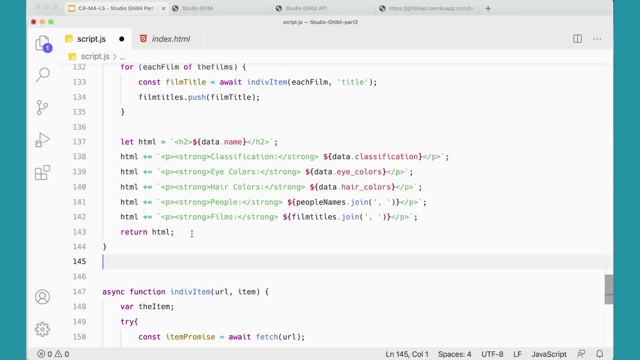 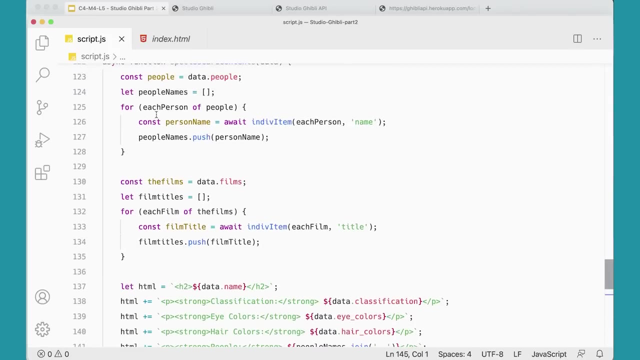 push those into the array. Same thing down here with film titles. Push that into the array and then print this, And then we're joining the people names and the film titles and returning the HTML. Nothing too fancy there. Okay, great, So there's that one. What did you get for vehicles? The vehicles one. 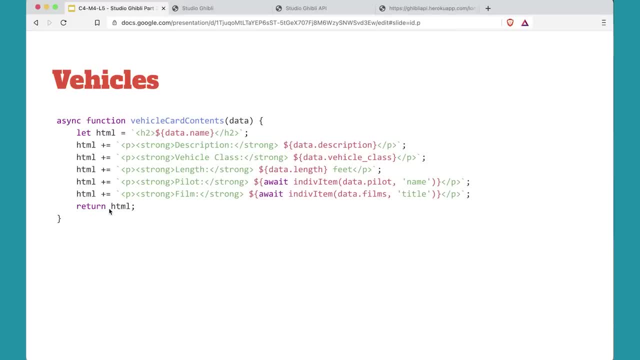 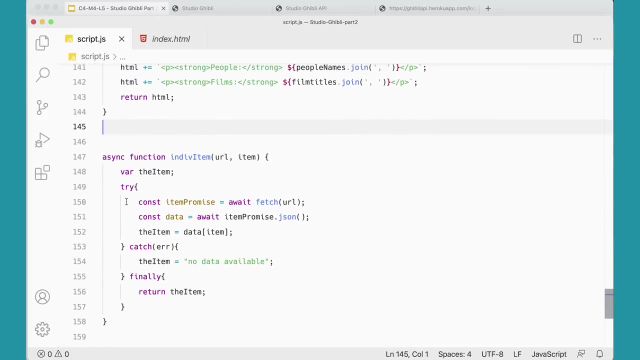 is shorter. We don't have that much, We don't have that many vehicles, We don't have that much information about vehicles, So it's shorter. So let's go ahead and add that one. Go back to my editor. Come down here. I'm going to add the vehicles here. 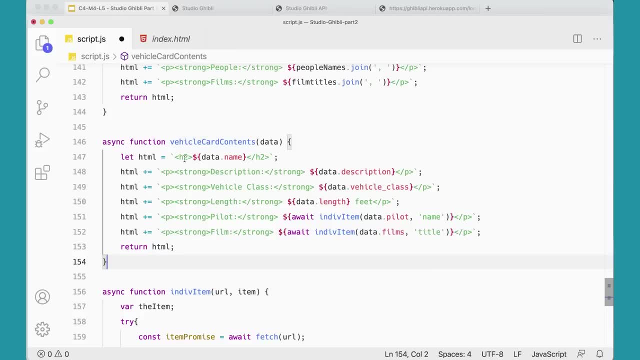 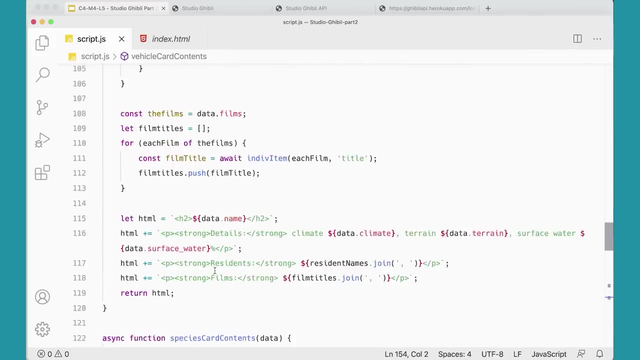 Leave my helper function at the bottom. So yes, this one is shorter and you'll see we don't have that many vehicles. That's fine. We've got that Now. the last thing that you needed to do was come up to this function up here and add some more cases. 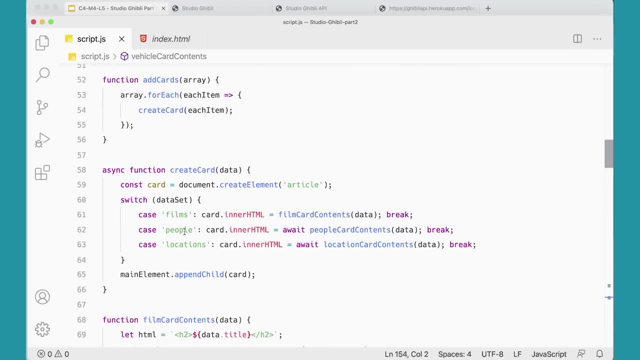 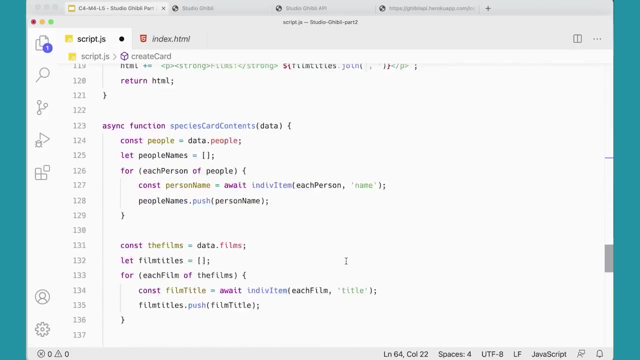 And here, where'd it go? This one here, I'm going to copy that. And this one is not locations, It was species. And then I need to get the species card content. I'm going to copy and paste the name of the function, just so I don't. 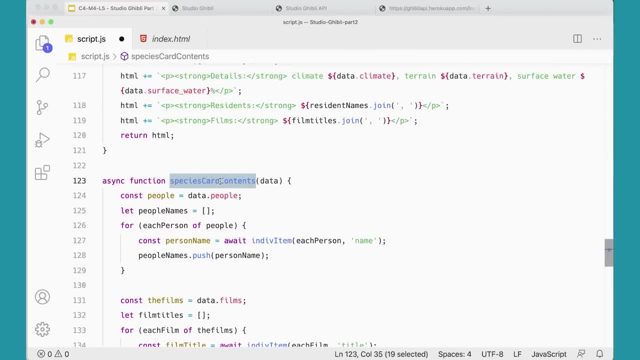 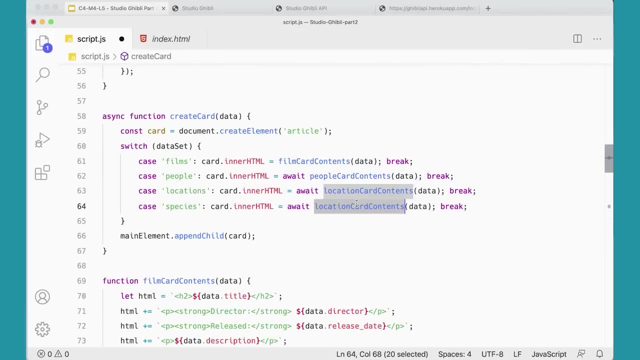 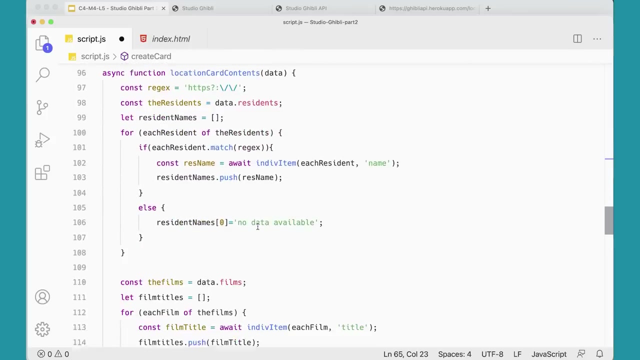 screw it up This one here. It's really easy to spell things wrong. So species card content. So we get that one And then the last one. If the case is vehicles, Okay, We're going to go down and get the vehicle card contents. 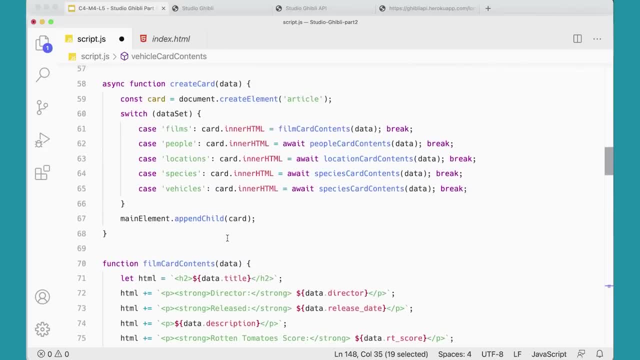 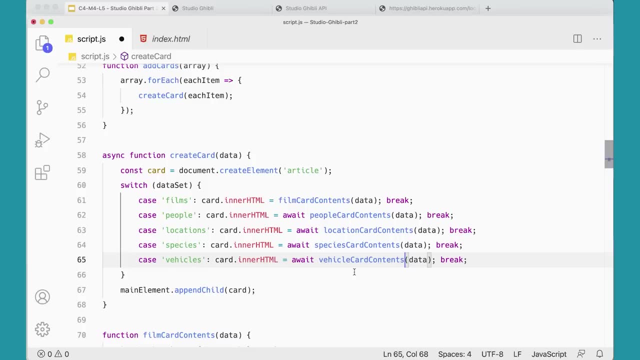 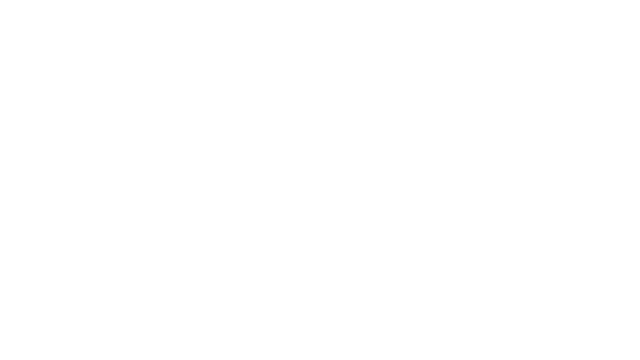 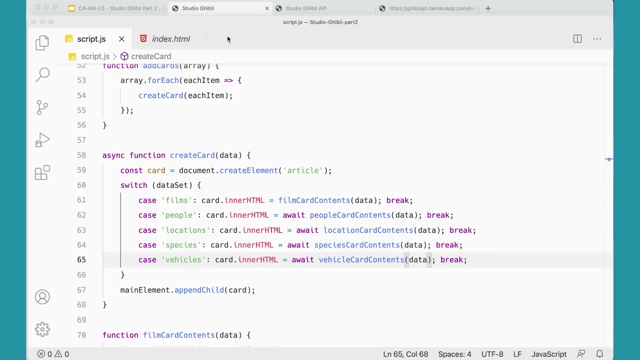 Sorry about all the scrolling in the video. There we go Save that. I think we've got that all right. Hopefully I spelled everything right And it's time to go see if we can test it. Come over here, I'm going to refresh my page. 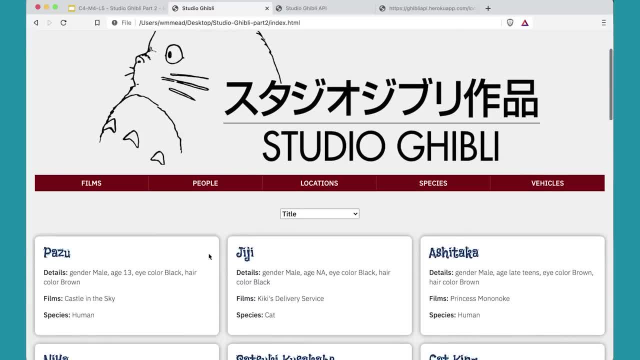 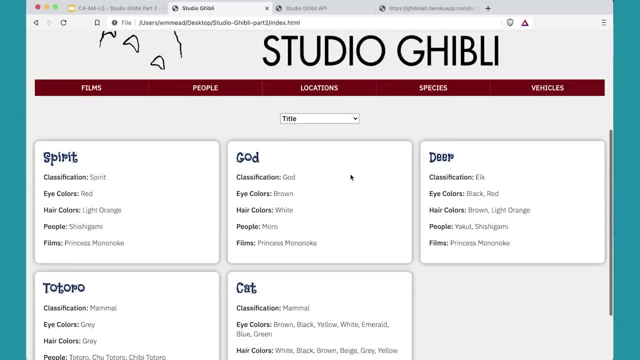 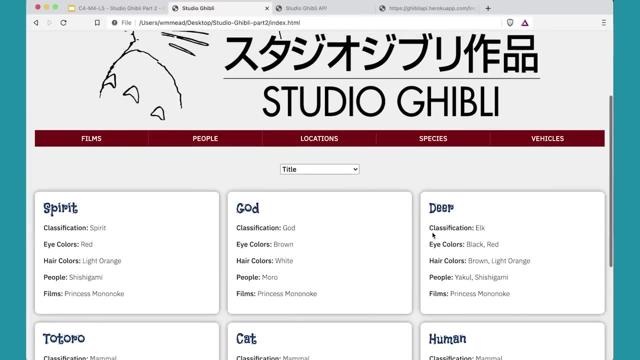 The films are coming up, The people are coming up, The locations are coming up, Big test species: They're coming up And it took a while for that to come in. You'll see why in a minute. And vehicles: We only have three vehicles. 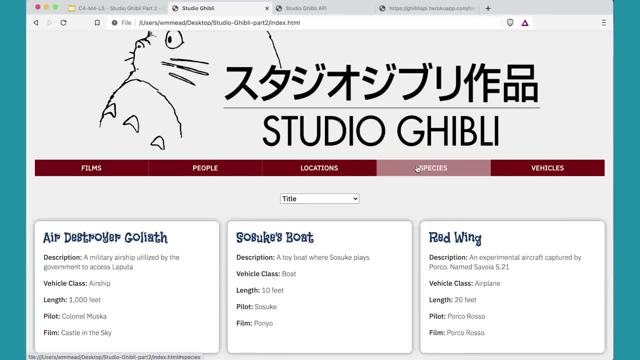 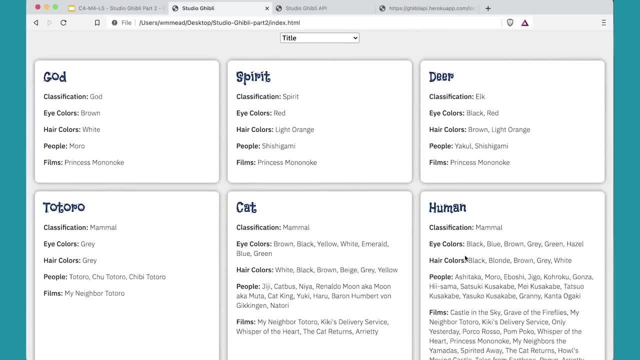 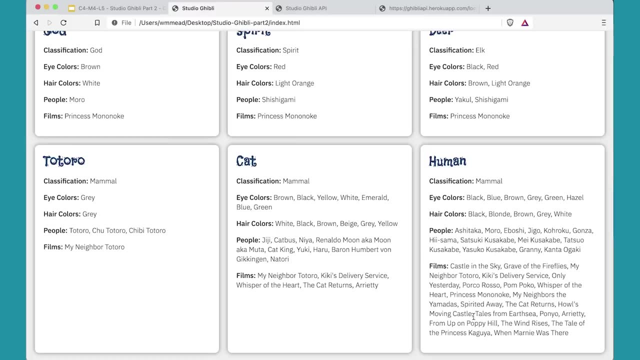 There's not that much there to get Now. it's interesting to note that when we do the species, it takes a while for the cat and the human to come up. because we're looping through all of this stuff, We're making a pretty big trip to the Asia. 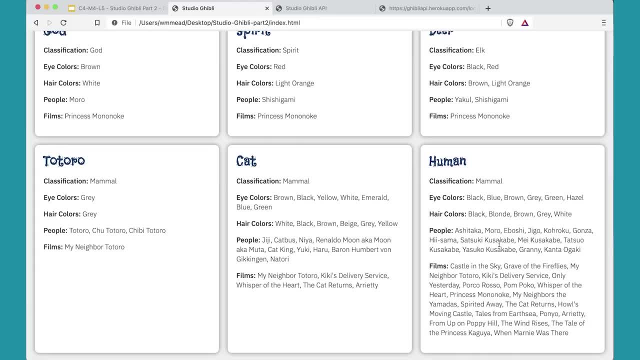 We're making a pretty big trip to the Asia to get all of this data for all of these films and all of these people here. So one thing to think about in terms of extending this project is: what could you do to keep this data local once you've gotten it once, so you don't have to go back to the API a whole bunch of times? 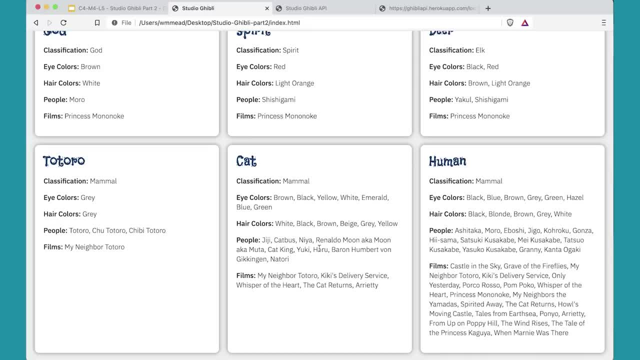 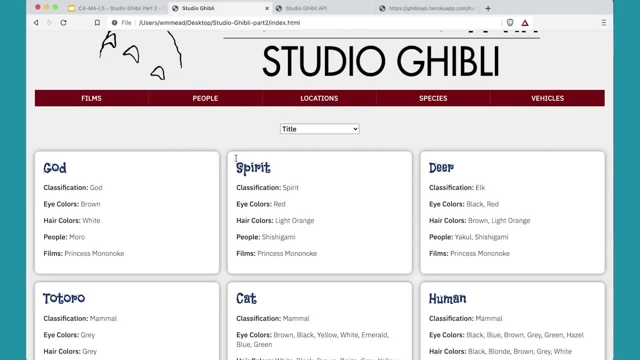 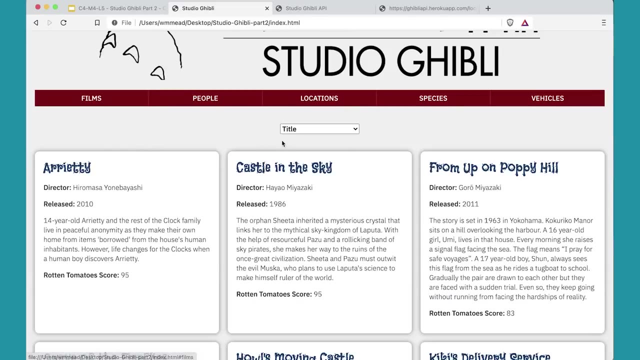 That would be a really interesting way of expanding this particular project is make it so. you don't have to do that Now. there's one last thing that I want to fix, which is this thing here: I really only want this to show up when we're on the films page, because that's the place where I can sort by these things. 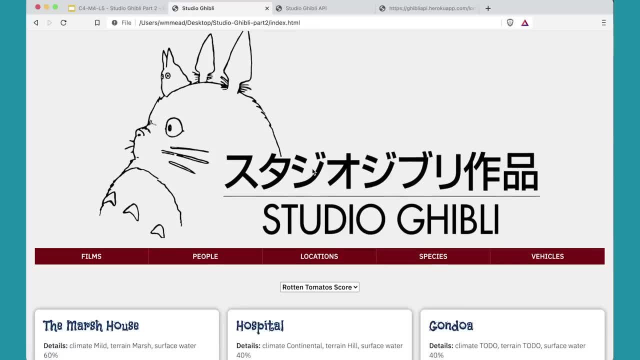 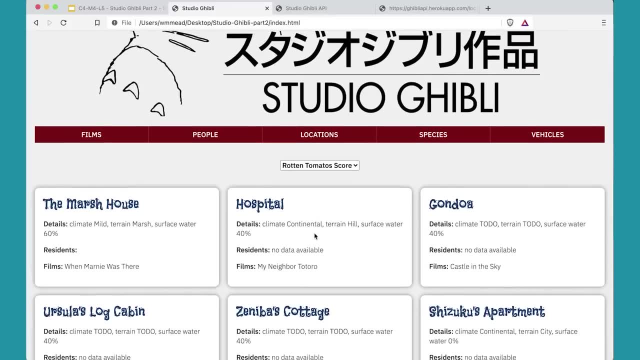 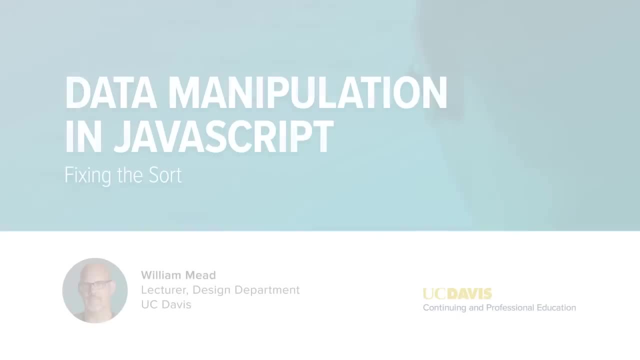 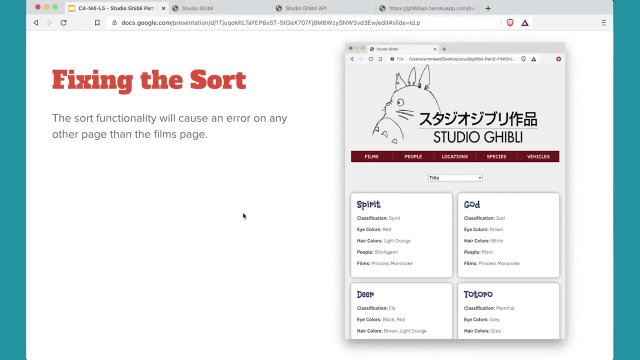 It doesn't make sense for that to show up when I'm on the locations page. I don't have a Rotten Tomatoes score on this page, So we'll fix that in the next video and then we're done with this project. The last thing to fix is the sort functionality. 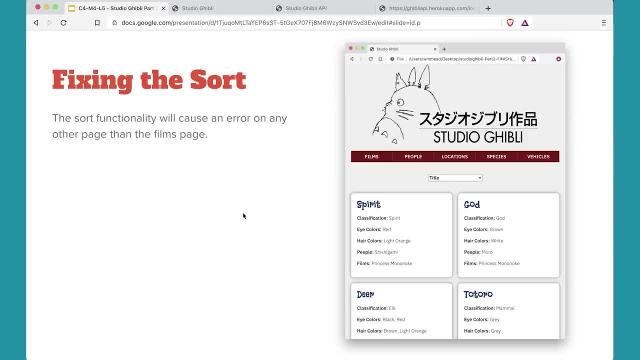 This sort functionality will cause an error on any other page that you use it on other than the films page. It'll only work on the films page, And one way to extend this project is to add an appropriate sort option for each page. That'd be something that you could look into and take on on your own if you're interested. 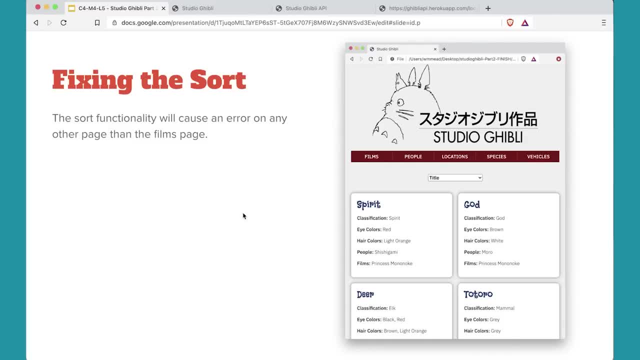 However, for the sake of this project, I'm going to go ahead and do that. I'm going to go ahead and do that. I'm going to go ahead and do that. I'm going to do that. At this point, we can just hide it on the pages that are other, on pages other than the film page. 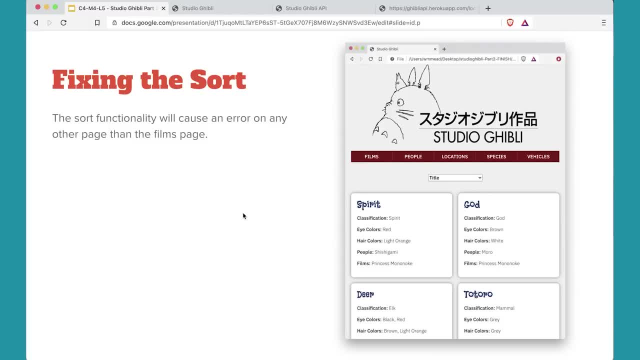 And here's a good challenge for you. There's a number of ways of doing this. Can you figure out one of them on your own? See if you can do it. Go ahead and pause the video. Go off and try it. See what you can figure out how to do. 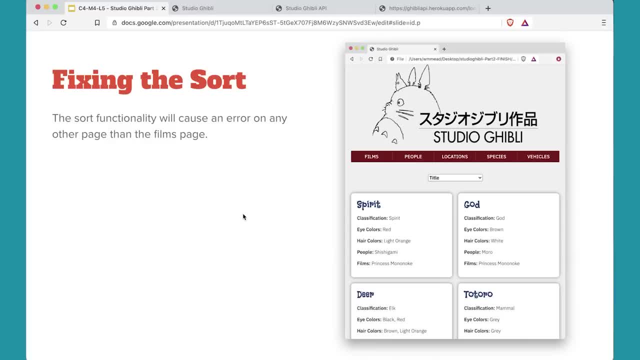 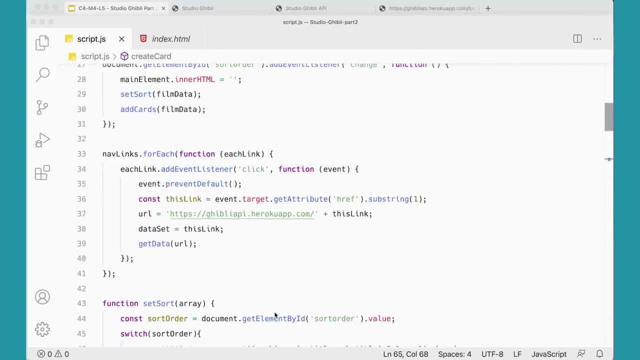 And then let me know, Come back and look and see how I did it. Were you able to do it? There's probably lots of ways of doing this. I'm going to show you how I did it. I'm going to go back to my function for get data. 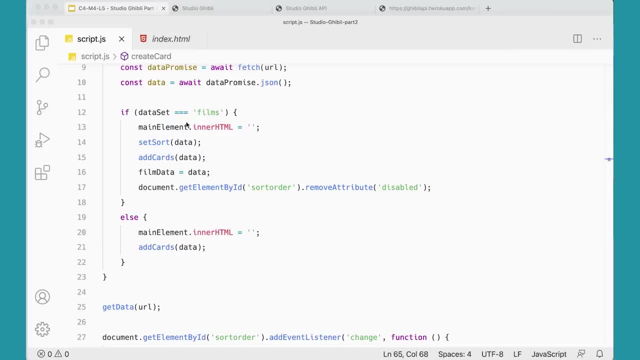 And when I come down here, to this part here, if I'm in films, I'm going to do this. If I'm not, I'm going to do that. Well, if I'm not in films, I'm just going to add in your document. query selector. 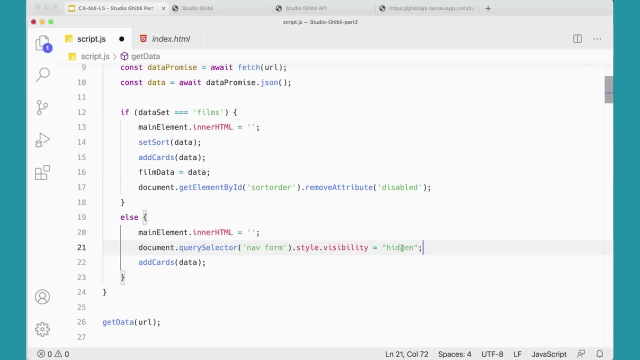 nab form style: visibility hidden and that will hide it if I'm on any other page. Now, if I'm on the films page, I also want to do the same thing. I'm going to stick it here, but instead change this to visible. 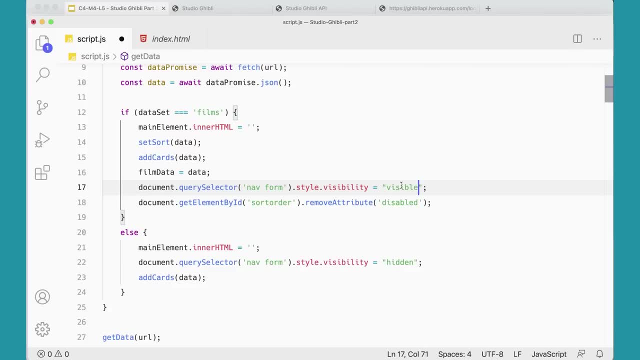 I like this method because the CSS property of visible and hidden means that it will take up the same amount of space on the web page. Even if it's hidden, the space will be there for it. So that means you won't have as much jumping between the content going from one. 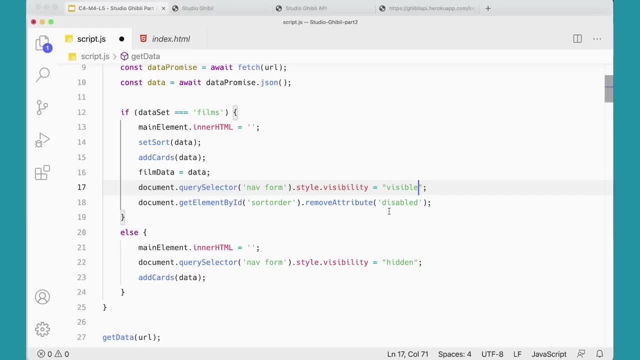 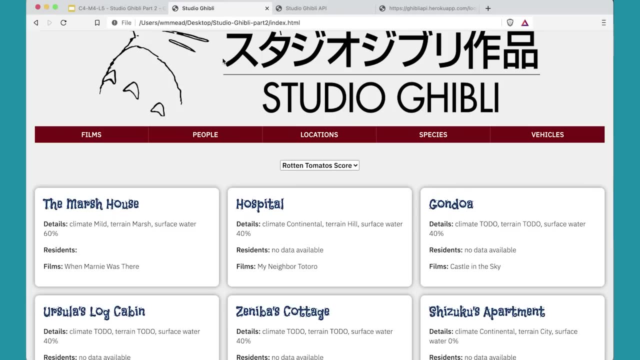 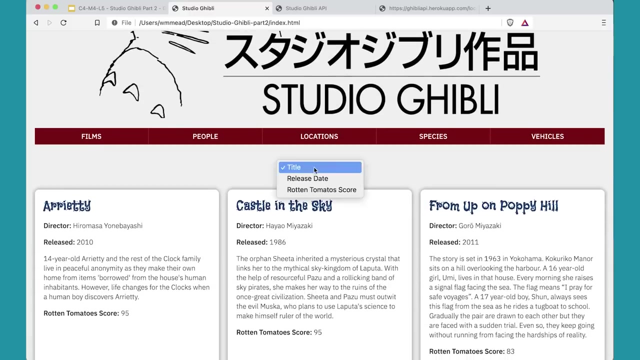 page to the next. So I kind of like that better in this case. Let's go over and test it real quick. If I refresh the page here, I am on the films page and it's showing and I can work with it and do all that kind of stuff. 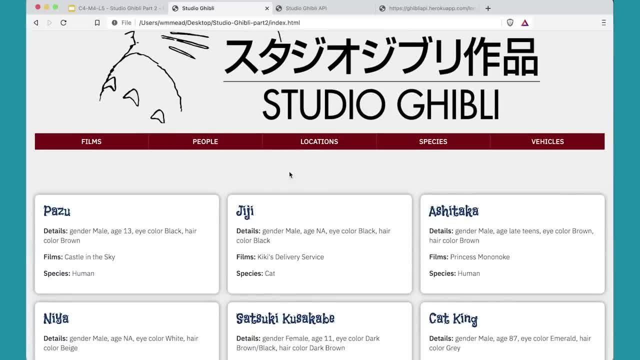 When I click on people, it comes up and it takes up the same amount of space. It's still there, It's just visually hidden, Um, so it takes up the same amount of space. So I have the same amount of space between here and there. 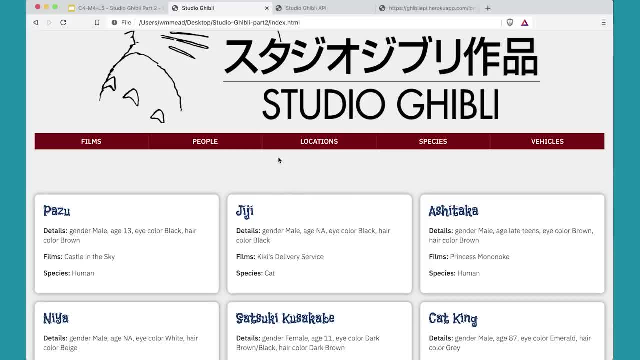 If I were, I could also set it to display none, but then that would take it off the DOM entirely and you'd have a smaller gap between the nav bar and the items coming up here. So I kind of like it that way. If I go back to the films page,